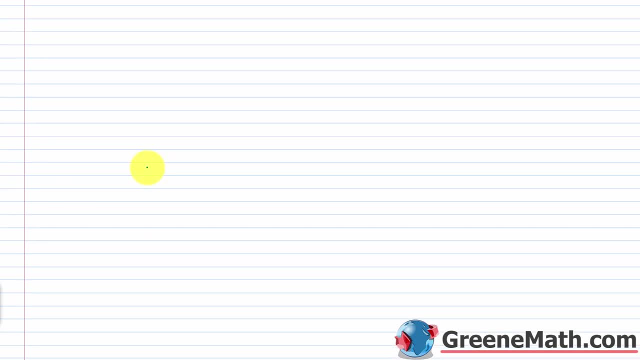 say a collection of numbers that fit a certain definition. So, as an example, let's start out by just thinking about the whole numbers. So this is a set or a collection of numbers that fit a certain profile. They start with the number zero and they increase in increments of one indefinitely. 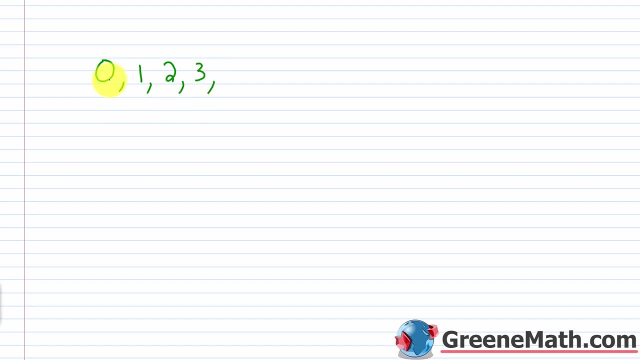 So, generally, when we list the whole numbers, we'll start with zero, we'll go 0123.. At some point we're going to stop because we can't list every whole number. that's impossible And we'll put three dots. Now we think about this. in regards to being a set, we have some more definitions. 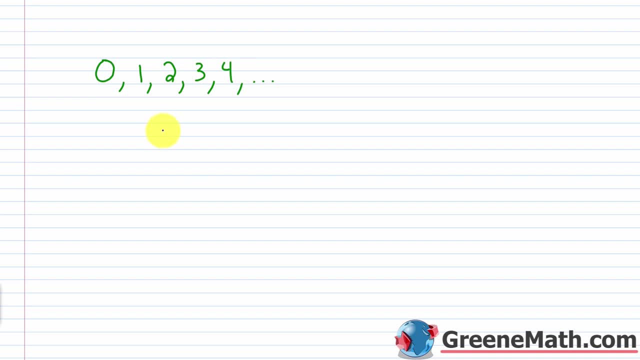 involved. So the numbers that are listed here are known as the members or elements Of the set And, like I said, it should be clear whether something is in the set or not in the set. So, as an example, if I asked you, is negative five a member of the set of whole numbers. 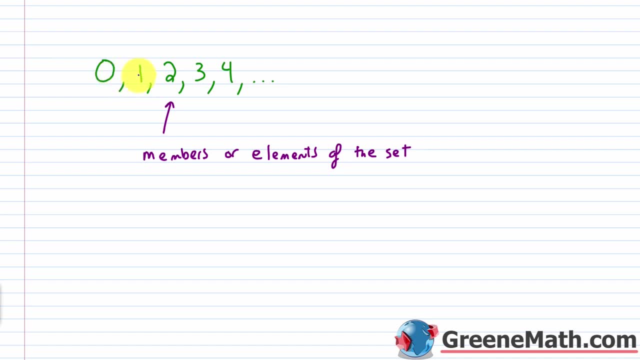 you would say no, because the whole numbers start with zero and increase in increments of one indefinitely. So that doesn't fit that profile or that definition. So it is clear that negative five is not a member of that set. Another thing that we do when we have sets: we enclose our members or elements inside. 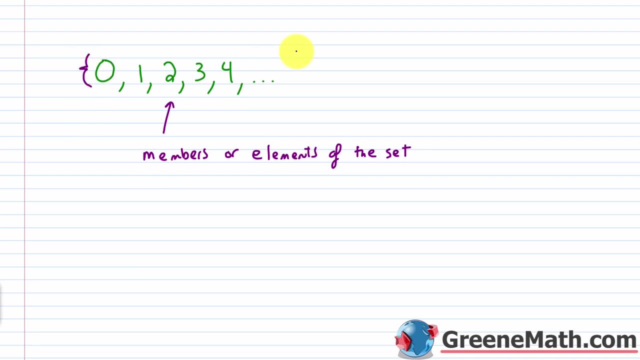 of set braces, So we're going to enclose this inside of set braces. So these are set braces, if you hear that. And the last thing I want to say here is that the method that we're using here is known as the roster method. 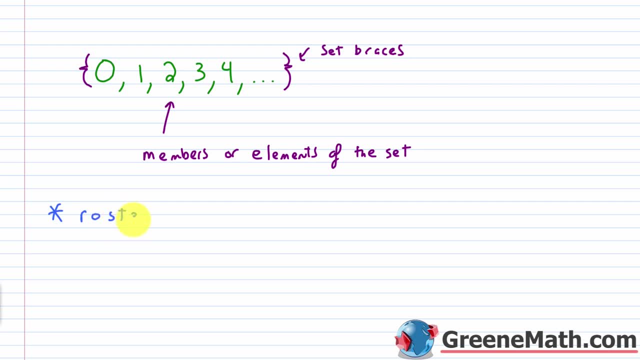 This is known as the roster method And basically what we're doing is we're listing the members or elements of the set inside of set braces. So that's the roster method. As another example, let's say we talked about the set of integers. okay, the set of integers. 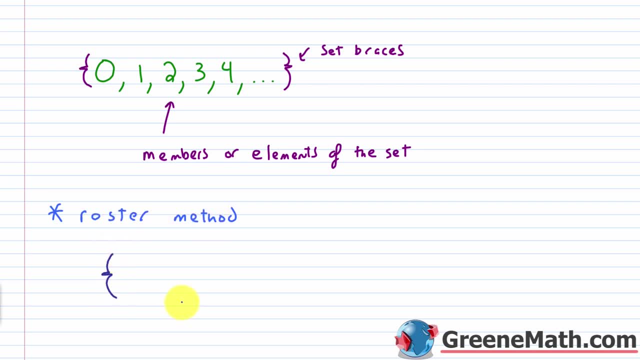 So the set of integers. if I use the roster method, again inside of set braces, I would have three dots coming this way. I'd start with a comma, I'd start with something like: let's say negative two, then negative one, then zero, then one, then two, then comma, and then again I'm going to put three dots. 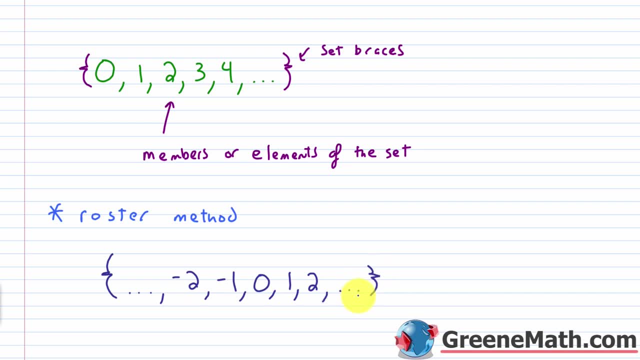 And again, in case you don't know what the three dots are, they're known as an ellipsis and they just tell you that the pattern is going to continue. So, going this way, I know that I'm decreasing by one. So after negative two, I'd have negative three, then negative four, then negative five. so 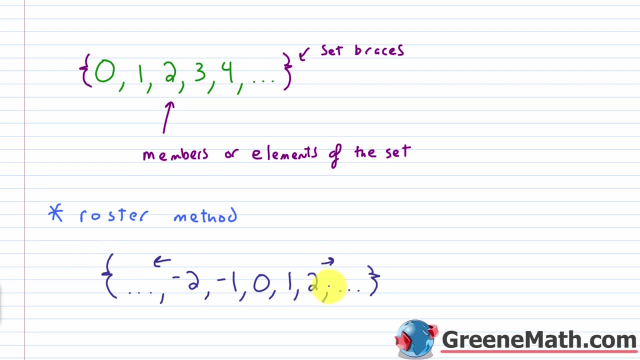 on and so forth. This way, After two I'd increase by one, so I'd have three, then four, then five, so on and so forth. So this is the set of integers, and again it's clear whether something's in that set. 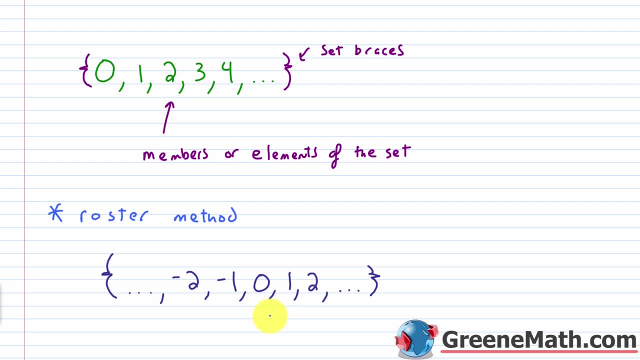 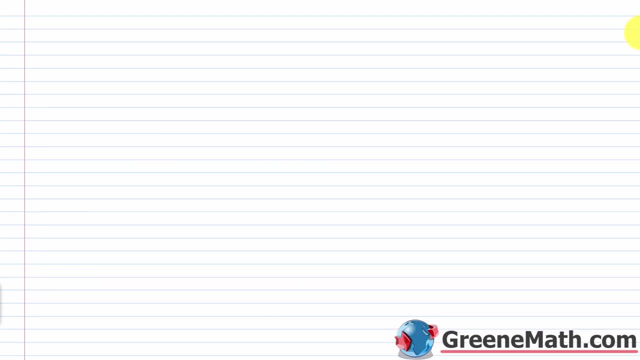 or not. If I gave you the number 0.675, it's clear that that's not an integer. It's not in that set. Now, although generally in algebra we're going to have sets that involve numbers, we can have sets that don't involve numbers. So let's say, as an example, I had a set that contained the first set of numbers, and then I had a set that contained the second set of numbers. So I'd increase by one, so I'd have three, then four, then five, so on and so forth. 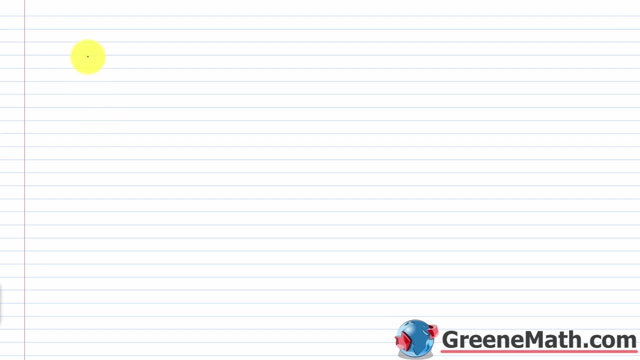 Well, again, if I had a set that contained the first five letters, then I'd have three, then four, then five, so on and so forth. Again, this is the set, of a set I'd increase by one, so I'd have three, then four, then five, so on and so forth. 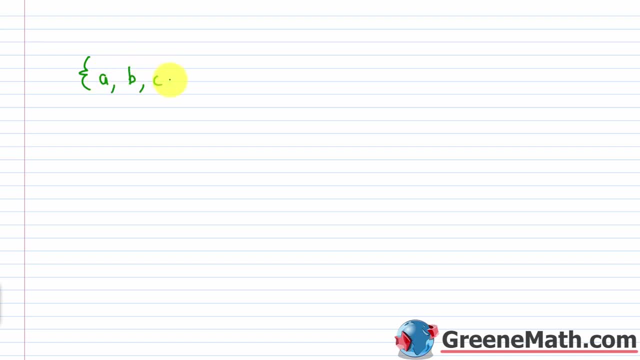 This is the set of a, set that contained the first five letters of the alphabet. Well, again, using the roster method, I would list a, b, c, d and finally e, the first five letters of the alphabet inside of my set braces. 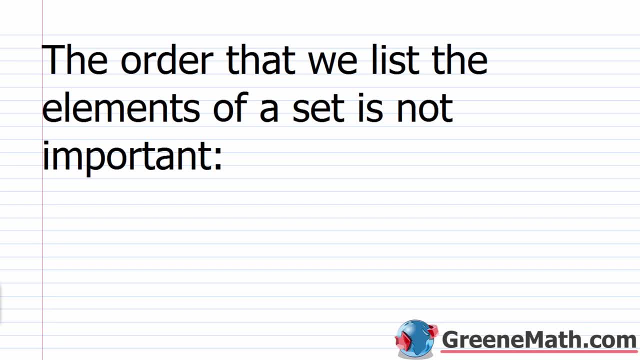 All right. so now that we have the basics under our belt, let's talk about a couple of other things. So the order that we list the elements of a set is not important. So let's say, for example, I have a set whose elements would be one, two, three. 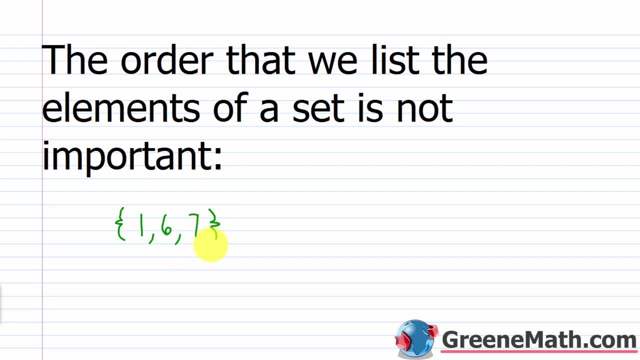 6, and 7.. This would be equal to the set whose elements would be, let's say, 6,, 7, and 1.. And it's also equal to the set whose elements would be 1,, 7, and 6,. you know as an example. 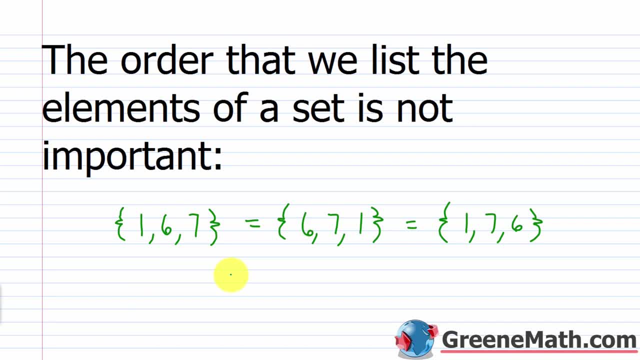 The order is not important. What's important are the elements or the members of the set. If this set contains 1,, 6, and 7, and this set contains 1,, 6, and 7, and this set contains 1,, 6, and 7,, they're equal because the members or elements are the same. 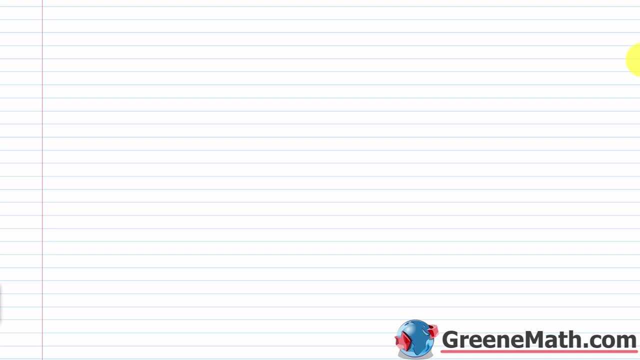 As another example of this, let's think about the states that border Louisiana. Okay, my home state is Louisiana, and so the states that border it are Mississippi, M-I-S-S-I-S-S-I-P-P-I- okay, kind of hard to spell- then Arkansas. 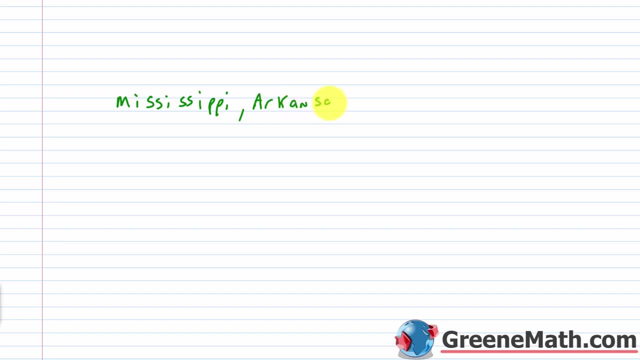 and and Texas. So this is the set whose elements are the states that border Louisiana, and this would be equal to the set with the same elements, just reordered. So let me reorder this. Let me write Texas first, then write Mississippi: M-I-S-S-I-S-S-I-P-P-I. 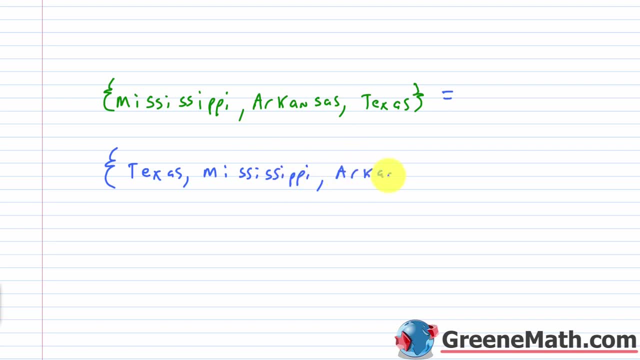 and then let me write Arkansas last And again. I could change the order as much as I want. What's important here are the elements or the members of the set. All right, so generally speaking, we can use capital letters to name a set. So we want to let A. 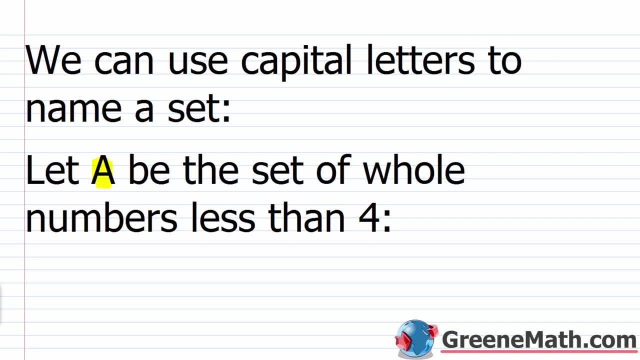 be the set of whole numbers less than 4.. So we know the whole numbers start with 0 and increase in increments of 1.. So I'll put a capital A out here and this equals inside of set braces. So again, the set of whole numbers less than 4 start with 0, then 1,, then 2,. 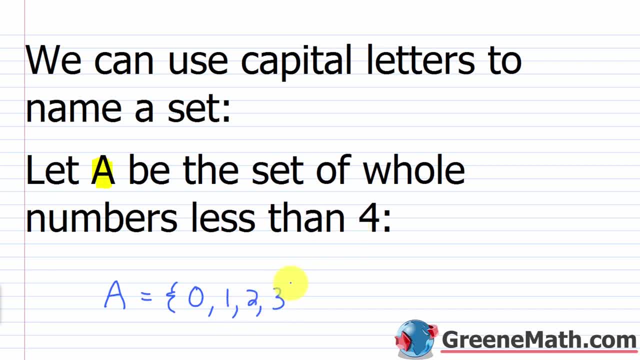 then 3.. It's less than 4, so I'm not gonna continue after that. So this is my set A Again. that's got the elements 0,, 1,, 2, and 3 involved, All right, So another big one that you need to know is: a set that contains no elements is referred to as an empty set, or 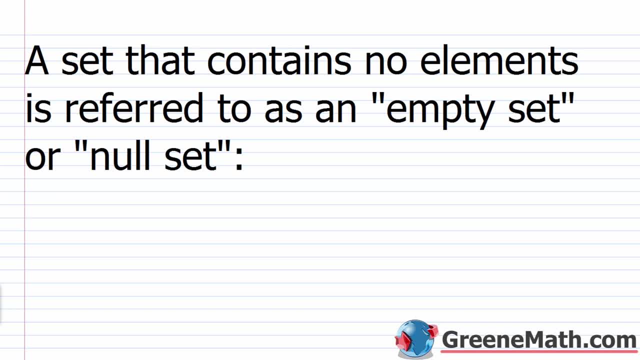 null set. So once we get into Algebra 2, we're gonna start using something known as solution set notation, and a solution set is nothing more than a set whose elements- elements- are a solution to your equation. So as an example real quick, let's say you had something like 2x minus 5 is equal to. 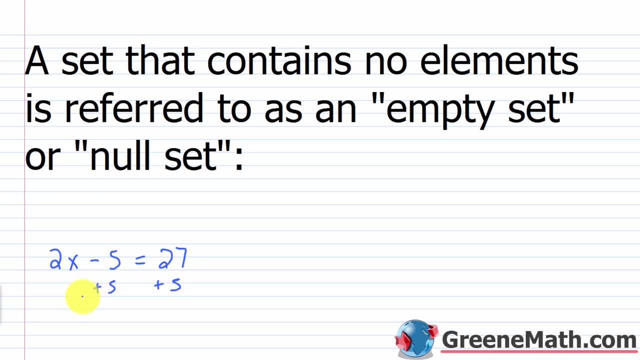 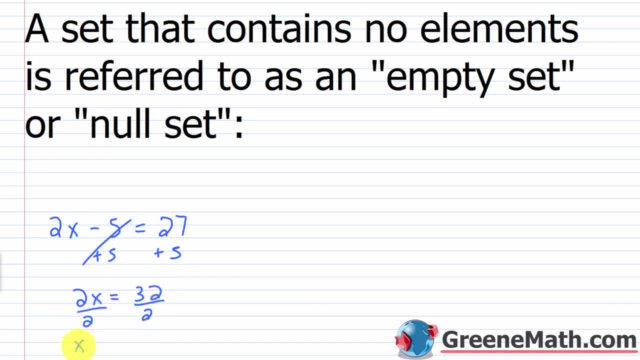 let's say 27.. So add 5 to each side of the equation- that would cancel- you get 2x is equal to 32, divide both sides of the equation by 2, you get x is equal to 16.. 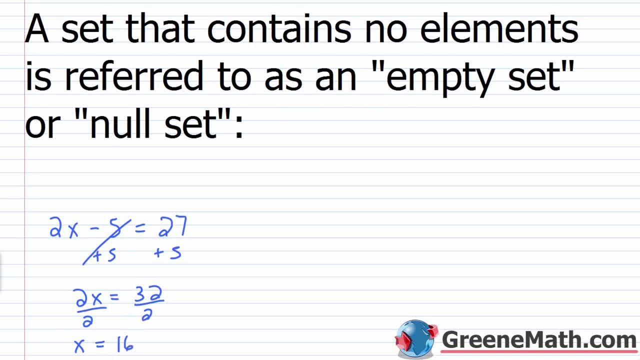 So to write this in solution set notation, I just literally put 16 inside of set braces. That's all it is. this is a solution set. This is a set whose elements are a solution to the particular equation that you're working on. 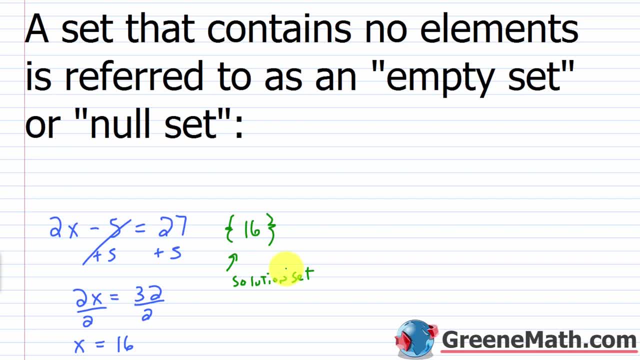 And this isn't particularly that useful when you get into Algebra 2, but if you get into higher levels of math where you solve something and you've got a bunch of solutions, it's just a neat and clean way to organize your solution. That's all it's used for. 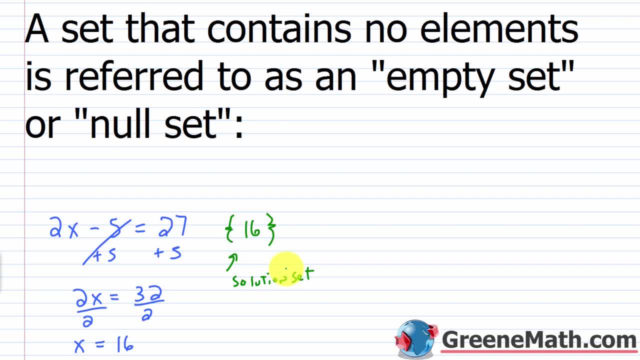 But we sometimes get equations that can't be solved. it'll have no solution involved. So a set that contains no elements is referred to as an empty set or null set. So what we're going to do is, if we have an equation with no solution, we're going to 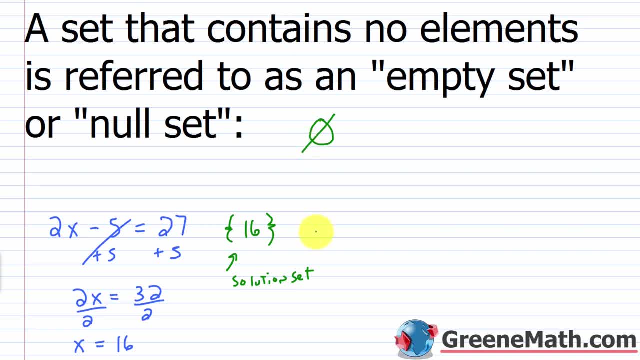 use this symbol right here to denote that Because that particular solution set has no elements. So if it has no elements it's the null set or the empty set. So you can use this symbol here for that, or you can also use set braces with nothing. 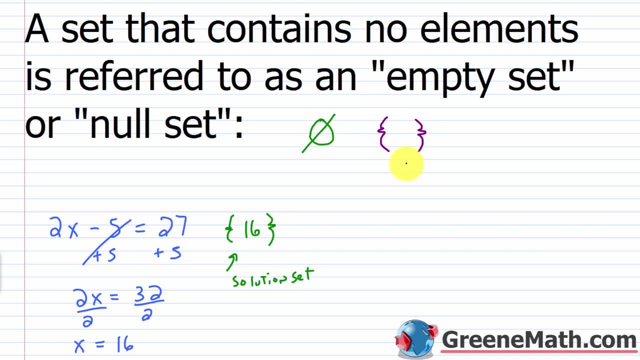 inside. But one thing I want to warn you of- and this is a big thing: when you get to college- math- do not do this. This is wrong. Okay, Write that down. It's a very common mistake that students make. Do not put this symbol inside of it. 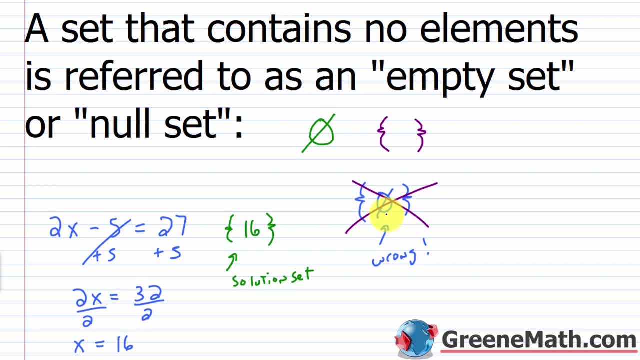 You don't want to do that. That is the set that contains one element and that element is the empty set. And I don't want to go into set theory and start confusing you, but just know that it's wrong, wrong, wrong. 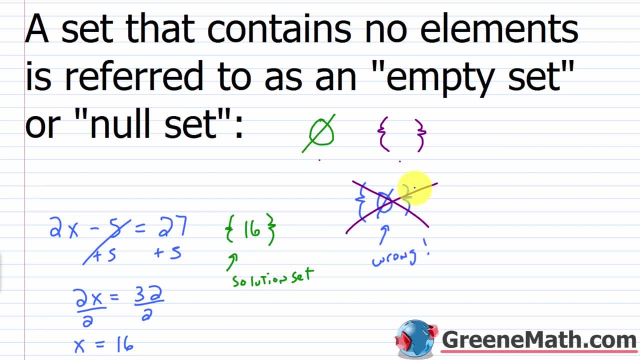 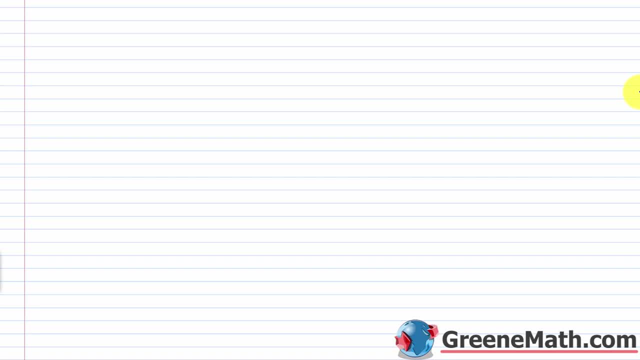 Okay, You can use this symbol, or you can use this symbol, but you cannot combine the two. So, as another example of this, let's say I said: let B. let B be equal to the set of all pigs that are living on set B. 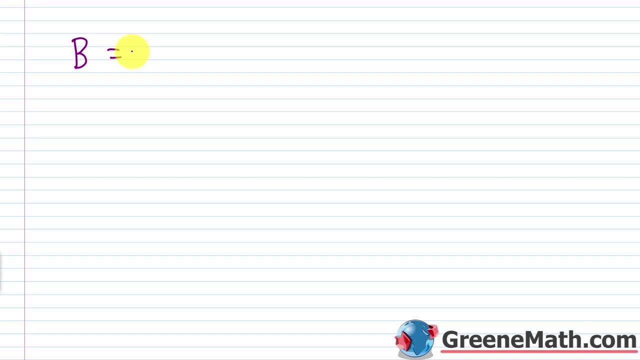 Now, I've never been to Saturn. chances are you've never been to Saturn, but I'm going to say that there are no pigs that live on Saturn. So that set would be an empty set, right, That set would contain no elements. 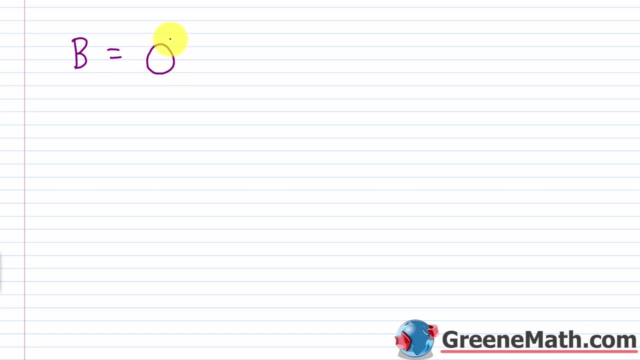 So we can say that this set can be denoted by the symbol for the empty or null set. or you could also say B is equal to this. But again, you cannot say that B is equal to inside of set braces. It's just a set. 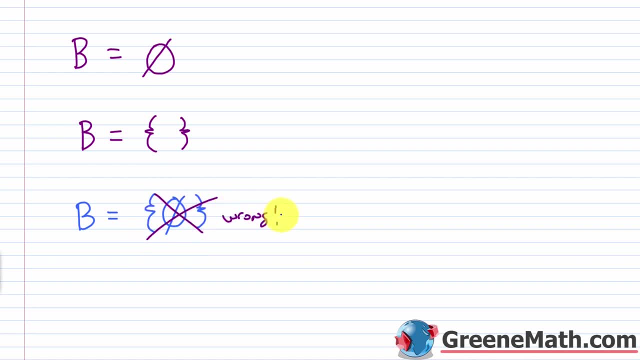 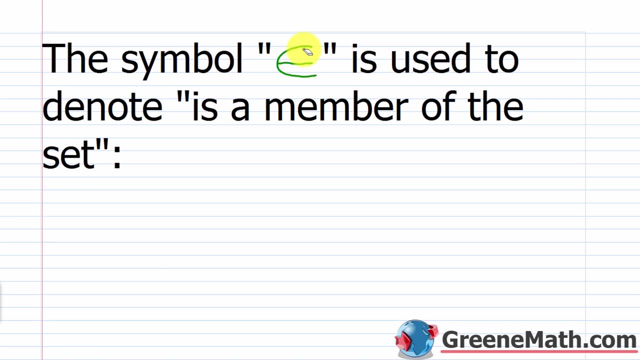 All right, And that Allison here, the P-U-L-E-S, that's the same as Z is equal to Z, Let's say that Z is equal to the set. Let's say we have Z and Z is equal to. Z is equal to, is equal to Z. 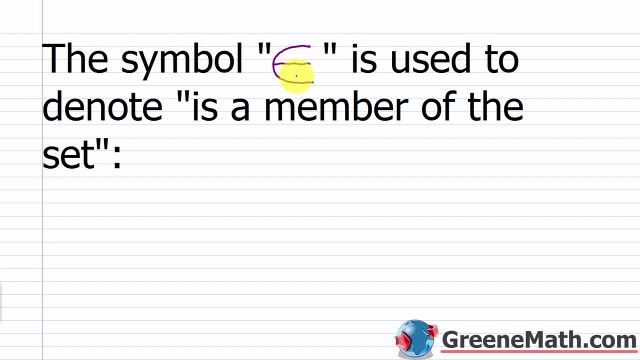 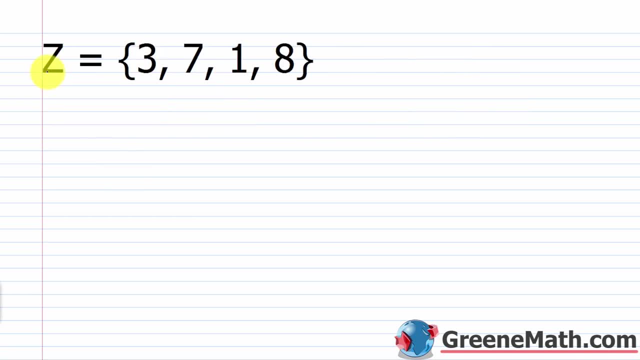 That's the set. That's where Z is equal to. So we can know that Z is equal to Z in the sentence and then we can say: oh, B is equal to Z in the sentence. Now let's say that Z is equal to Z in the sentence. So the second thing to be able to do- and this is again a case where I want you to know, but this is the thing You can see- that B is equal to B is equal to Z. Say that it's equal to Z. 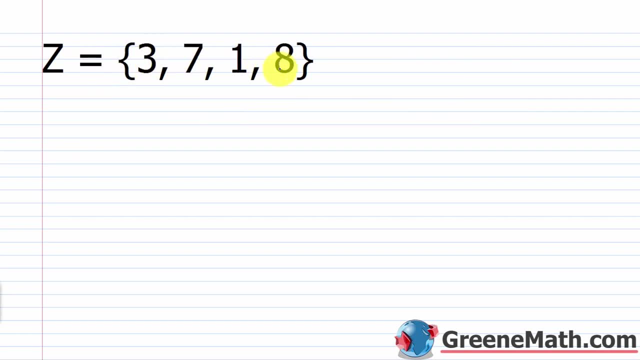 the members 3,, 7,, 1, and 8.. So what I can do is I can take each one and I can say, okay, 3 is an element of set Z, It's denoted like that. Or I could say: 7 is an element of set Z, Or I. 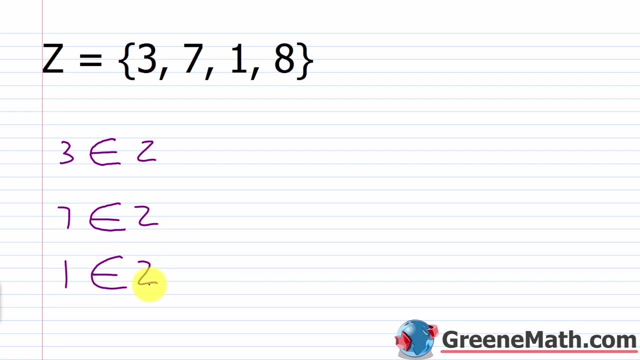 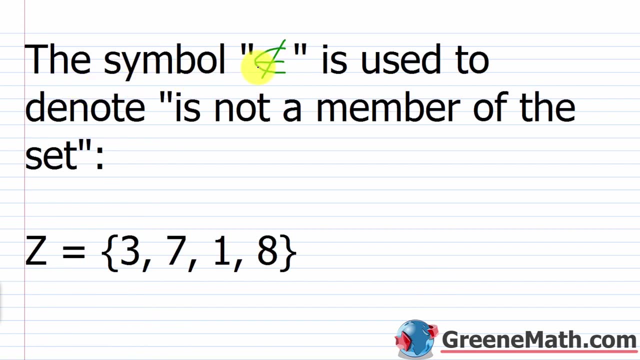 could say: 1 is an element of set Z. Or, lastly, I could say: 8 is an element of set Z. Now, similarly, the symbol here- basically we just put a line through, the other symbol is used to denote- is: 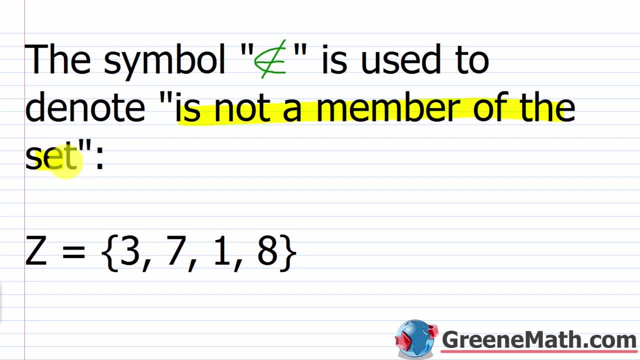 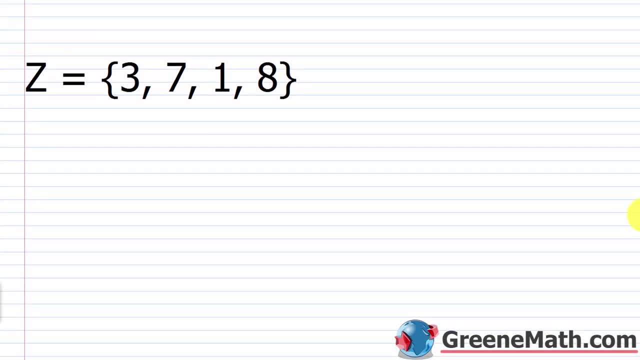 not- let me highlight that is not a member of the set. So with the same set Z, with the members 3,, 7,, 1, and 8,, I could do something like this. I could say something like: 6 is not an element. 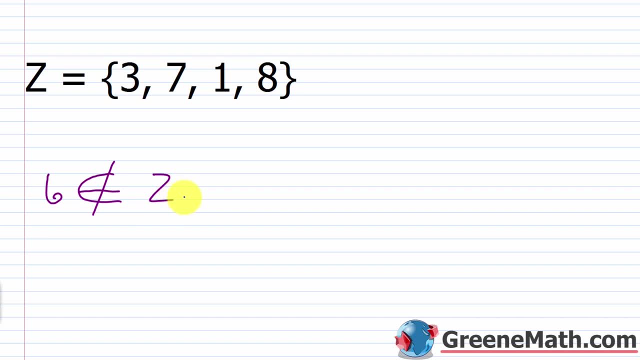 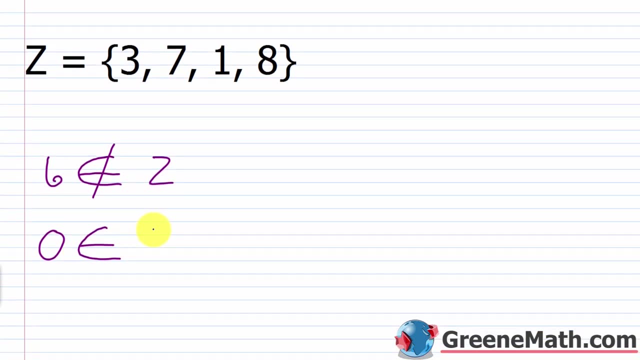 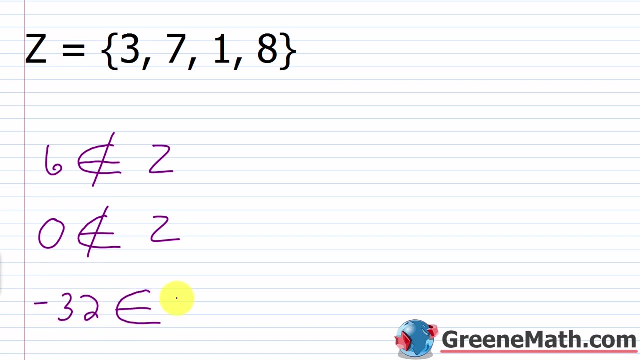 of the set Z. I could really use anything I want other than these four numbers. I could say 0 is not an element of set Z. I could say negative 32 is not an element of set Z. You know so on and. 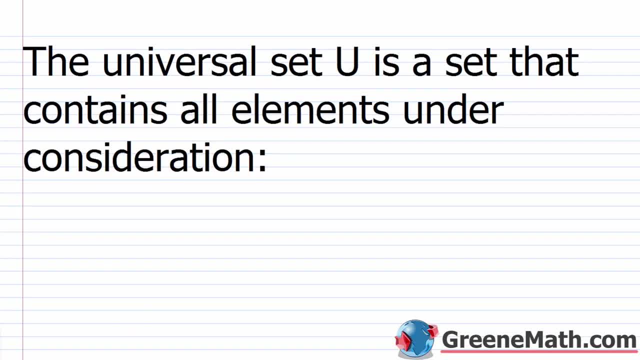 so forth. So another important concept would be that of the universal set. So this one's a little bit difficult to wrap your head around at first, but something after you practice a few of these that you really can understand. So the universal set, which is generally denoted with a capital, 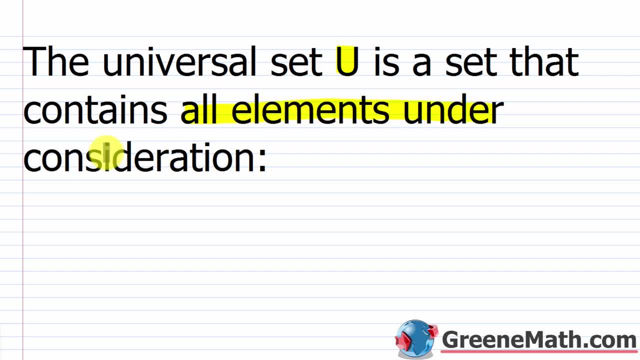 is a set that contains all elements under consideration. Now, if we're talking again about the states that border Louisiana, let's just name this. for the purposes of this example here, Let's name this as set A. So set A has the elements that fit this profile where they're. 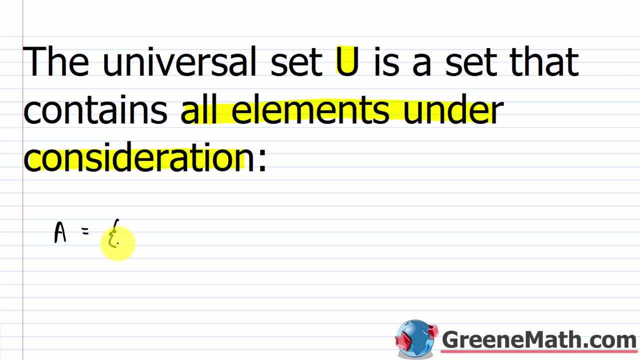 states that border Louisiana. So we already know that this would be Mississippi, M-I-S-S, I-P-P-I, We know it would be Arkansas And we know that it would be Texas. Okay, so three elements in this set. But if we think about the universal set here, what are all elements under? 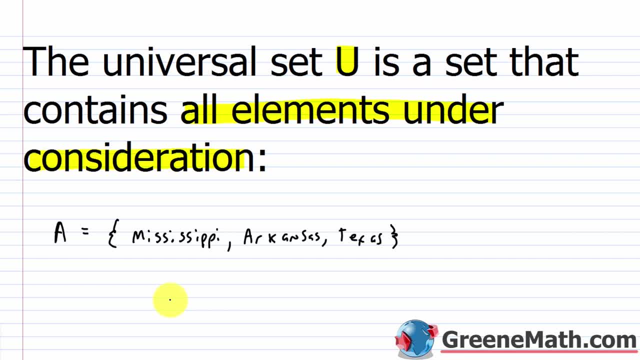 consideration. Well, we're talking about states in the United States of America, So all elements under consideration would be all of the states in the United States of America. So the universal set would contain every state. Now, we're not going to list all of them, That would be very time. 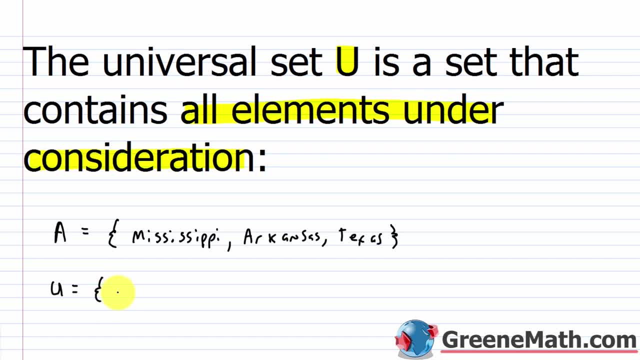 consuming, But in alphabetical order, we could just start with two of them. So in alphabetical order, it would be Alabama, Then it would be Alaska, And let's put our three dots there And let's finish up with the last two, which would be Wisconsin And then Wyoming. 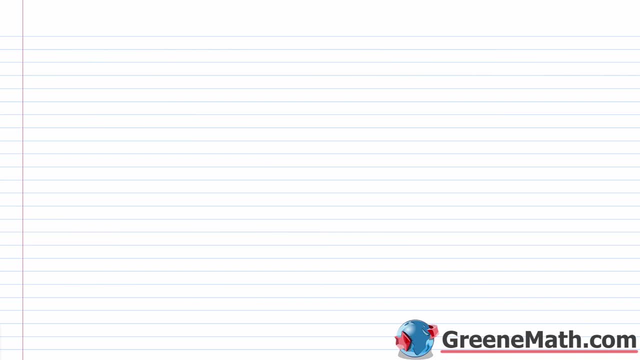 Now, as another example of the universal set, let's say we're again talking about the United States, So the United States has a president, We all know this. And we could talk about a set- and let's call it set A again- whose elements are the presidents that are currently living. 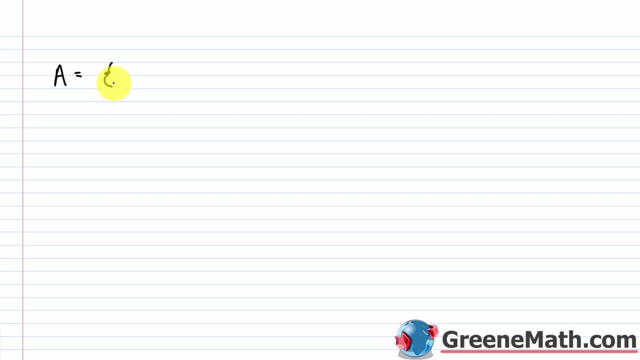 Now this set would change over time. We're filming this video in 2015.. So in 2015, the living presidents: we would have Jimmy Carter, We would have George Bush Sr. So let's just put G period, B period, And we'll put number one. 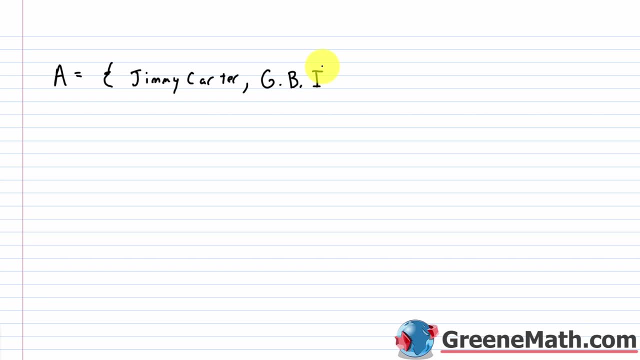 because he was the first George Bush to be president, Of course his son would be George Bush II. So then comma. After him we have Bill Clinton, And then comma, We're going to have George Bush number two, or George Bush. 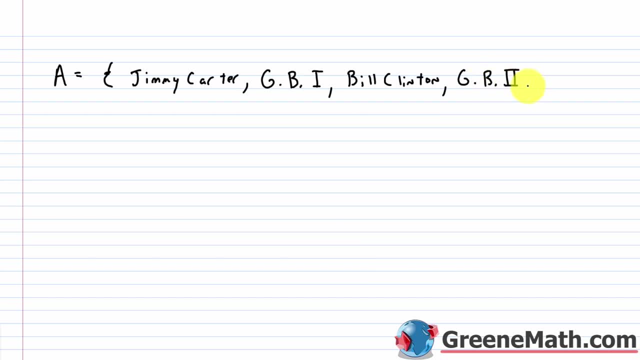 So G period, B period, and then two, And then we're going to have Barack Obama And, to fit this on the screen, I'm just going to put B period, O period, And then we're going to close up with some set braces at the end. So these are all the living presidents as of 2015.. Now, in 2016,, 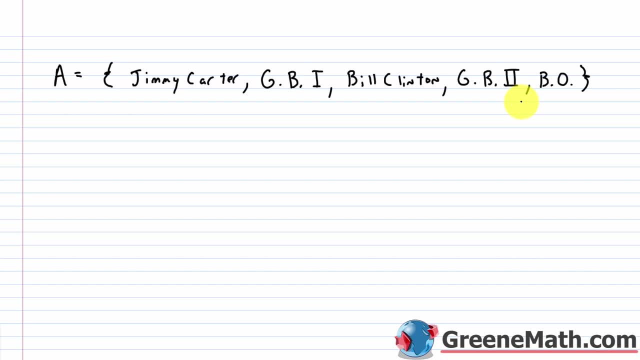 we're going to have a presidential election, So for sure it's not going to be Barack Obama, because he's going to be out of office. So we'll have a number of presidents that are going to be out of office. We're going to have another president to add to this list, But as people pass away as new presidents, 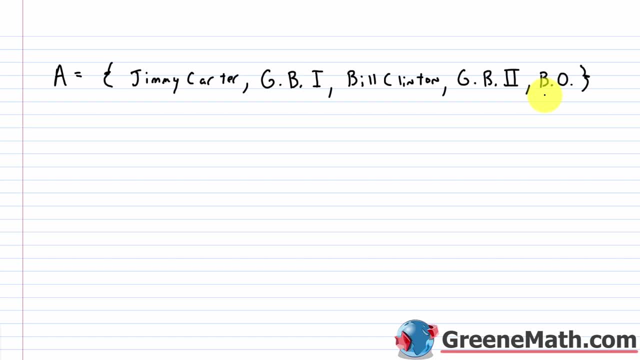 get elected. this set would change over time, But what's important is to understand that the universal set, the set with the capital letter U, would be what It would be all of the US presidents that ever existed. So we would start with George Washington. So George Washington. 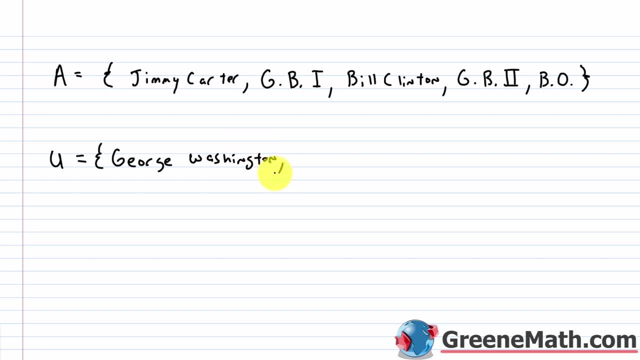 And then the next one was John Adams, And then, of course, after that you had Thomas Jefferson and so on and so forth. So let's just put three dots here And we'll kind of come in with the final two. We had George Bush, number two. 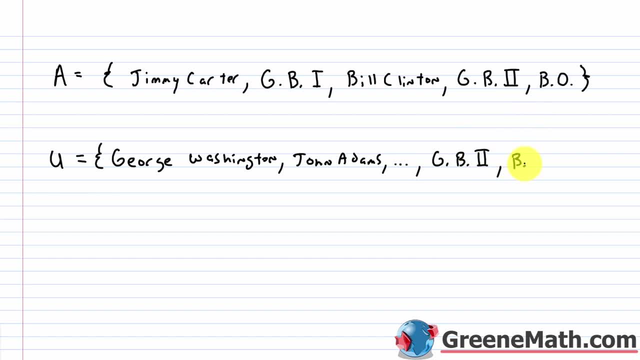 or George Bush Jr. And then we had Barack Obama, And again it could be whoever in the next election that wins. So this, this would be added to: If Donald Trump wins, If Hillary Clinton wins, If you know somebody else wins, We'll have another president to. 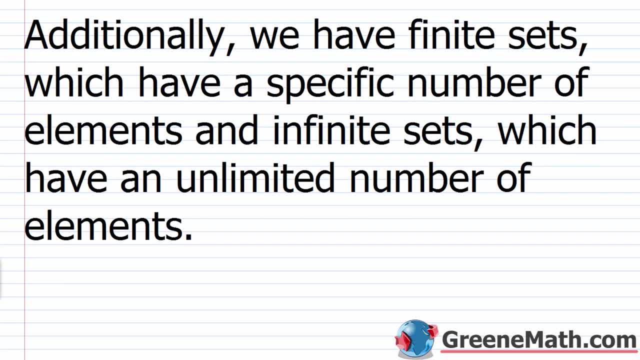 add to both lists, Alright. so, additionally, we have finite sets, which have a specific number of elements, And we have infinite sets, which have an unlimited number elements. So, as an example of a finite set, let's say I told you that we had a set A. 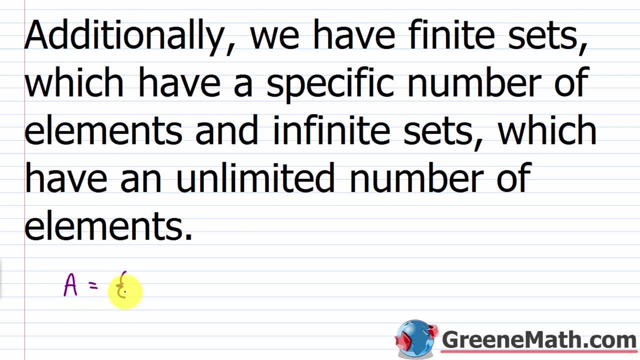 which was the whole numbers that were less than 6.. So this would be 0,, 1,, 2,, 3,, 4, and then 5.. So that's a finite set. I can count 1,, 2,, 3,, 4,, 5,. 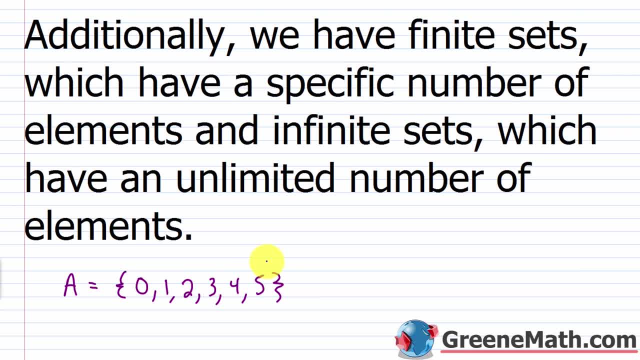 6 elements involved there. But if I said, give me the set of whole numbers or give me the set of numbers that are larger than, let's say, 5. Those are each infinite sets because they go on forever and ever and ever and ever, You can't possibly count them. Okay, so that's an infinite. 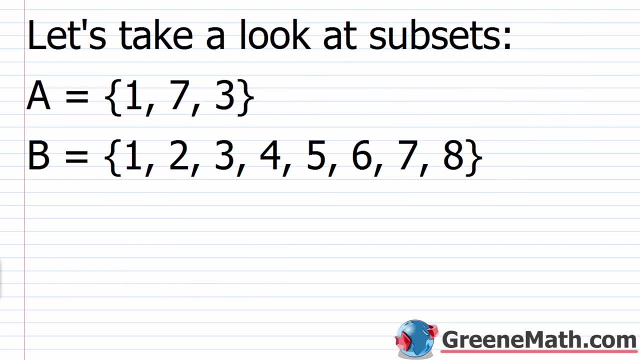 set. All right, so let's wrap up the lesson by talking about subsets. So this is something that you might get tested on, Kind of. the other stuff we looked at was just kind of you know, basic definitions, But these are things that you might have to think about a little bit, So let's take 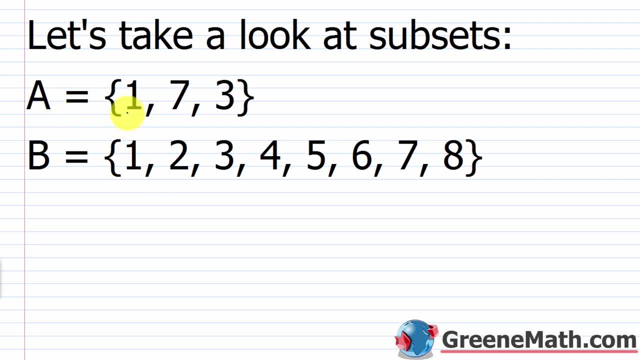 a look at subsets. So if I have set A, which contains the elements 1,, 7, and 3, and set B, which contains the elements 1 through 8, then A is known to be a subset of B And, more specifically, 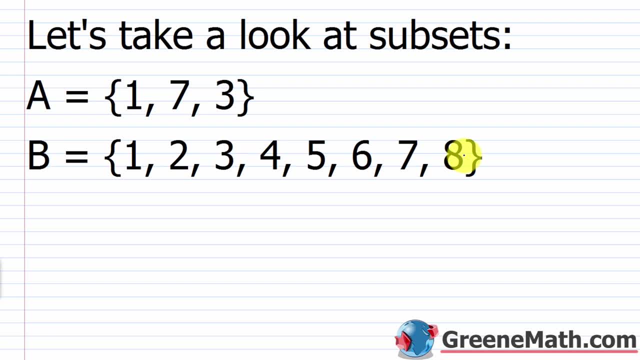 A is a subset of B. So if I have set B, which contains the elements 1,, 7, and 3, and set B, then A is a proper subset of B, because B contains all elements of A and they're not equal to each. 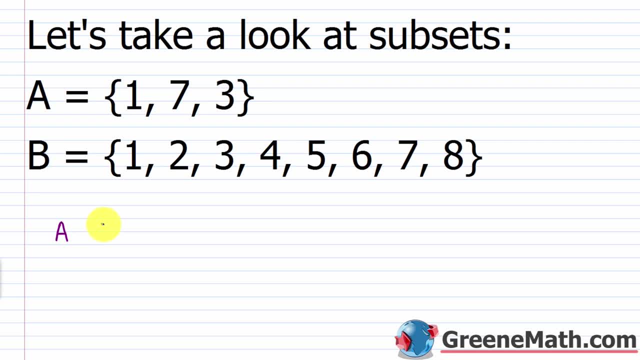 other. So A is a subset or a proper subset of B, And a lot of times this gets confusing because you have A and you have B And this kind of looks like a- C. So let me just take a look at this. So if I have set B, which contains the elements 1,, 7, and 3, and set B, 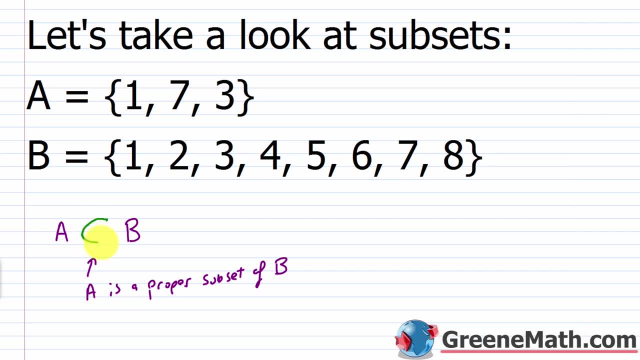 let me make it a little longer. I'll also do it in a different color. Let me do that So it kind of looks like a C, But that is a symbol for is a proper subset of. Again, if you look at B, it's got. 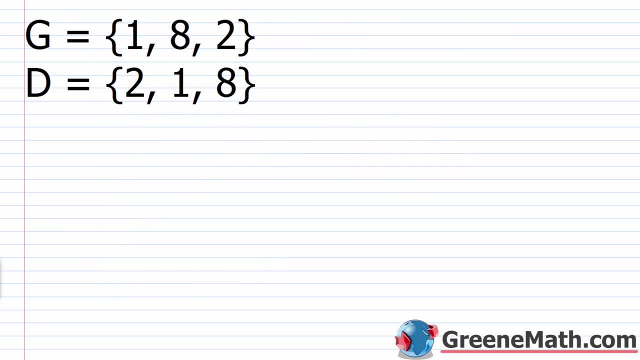 1,, it's got 7, and it's got 3.. Now if two sets are equal, meaning they have exactly the same elements, they're known as improper subsets of each other. So in this example we have G, which has 1,, 8,. 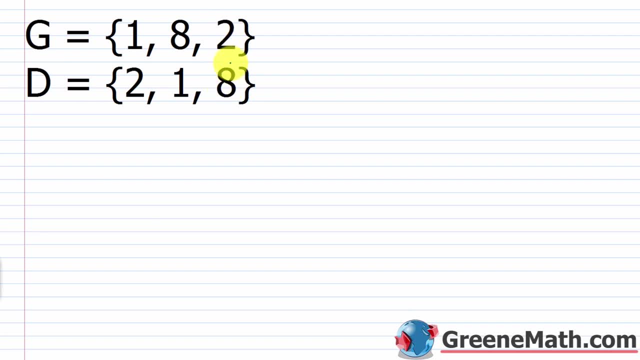 and 2, and D, which has 2,, 1, and 8.. These two sets are equal to each other because they have the same elements: 2 and 2,, 8 and 8,, 1 and 1.. So the exact same elements, so they are equal. So we can say they are improper subsets of. 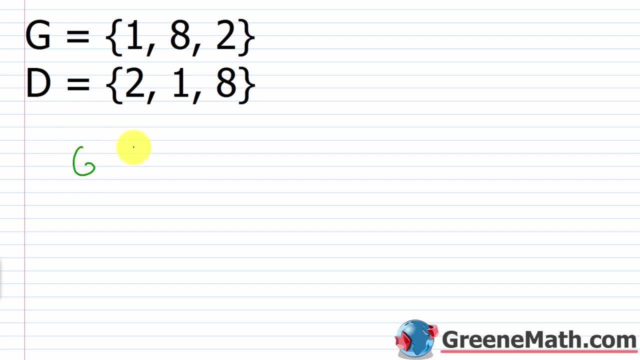 each other. So we show that by saying G is an improper subset- See that little bar- is an improper subset of D. And then also you could say: D is an improper subset of G. And let me just label this: This is: G is an improper. 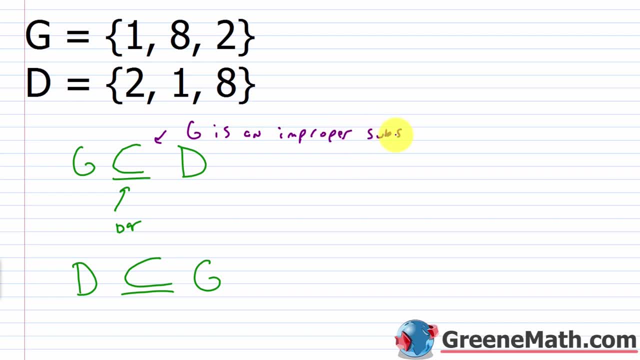 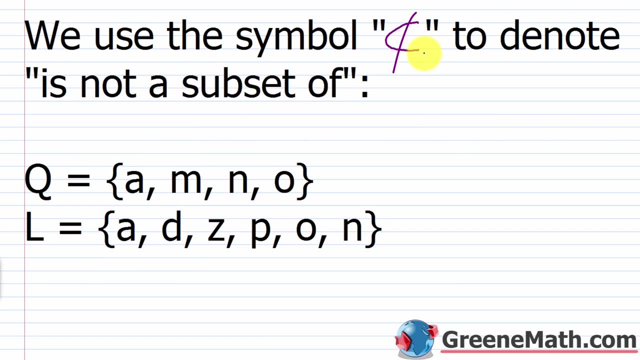 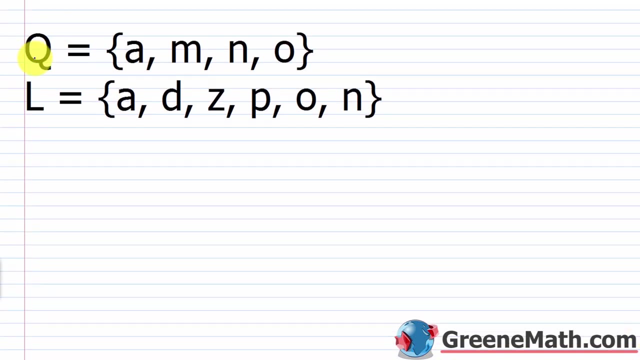 subset of D. All right, so we use the symbol here to denote is not a subset of, So it's just the proper subset symbol with a line drawn through it. So as an example, here we have these two sets. We have Q, which has A, M, N and O, We have L, which has A, D, Z, P, O and N. So we'd ask the 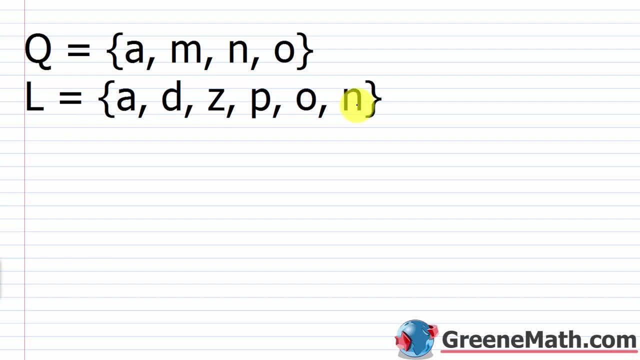 question: is Q a subset of L? Well, no, it isn't, And the reason it's not. this has A and this has A. This has M. This doesn't have M, So no M. This has N and this has N. And then this has O and. 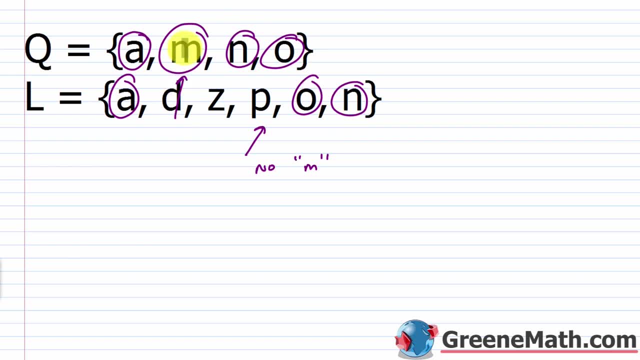 this has O, But because it's missing this M here. it's not a subset. For something to be a subset of another, it's got to contain all of the elements. You can't be missing something. So Q is not a subset of L. Q is not a subset of L. But if I was to change this set and let's say I: 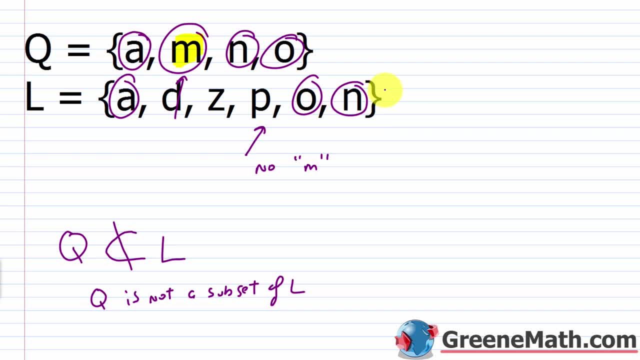 was to put an M in there, then it would be a subset, because L would contain all of the elements of Q. So that's what we mean here when we say Q is not a subset of of L. So, lastly, let's discuss how many subsets can be made from a given set. Well, the answer. 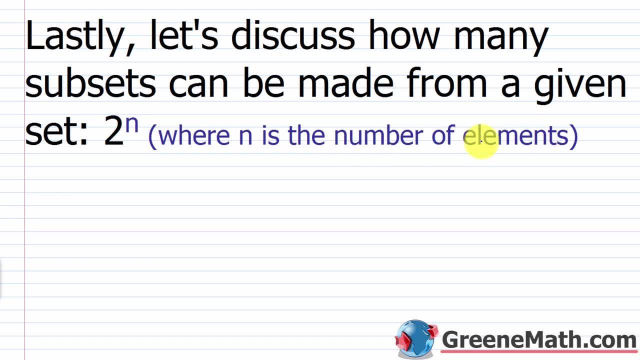 to, that is 2 raised to the nth power, where n is the number of elements that we have. So, for example, if I have, p is equal to, let's say, 5,, 7, and 9.. Well, the number of subsets. 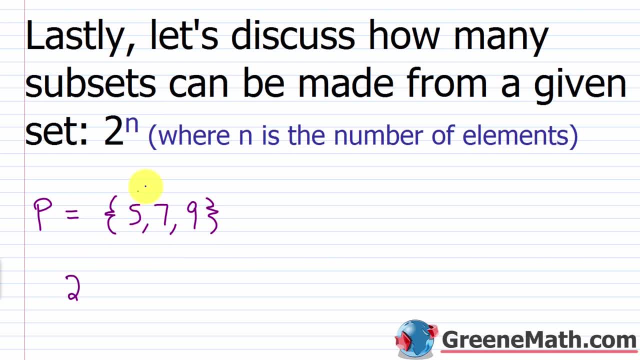 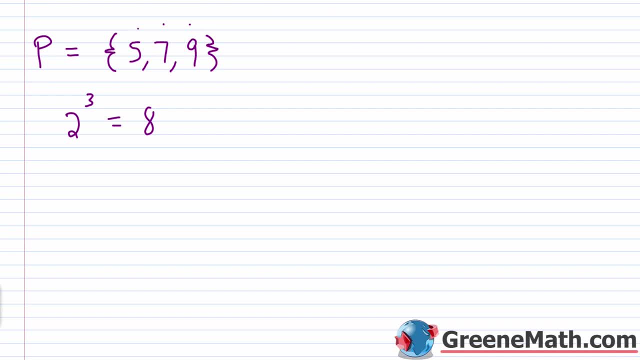 that can be made from this is 2 raised to the power of 1,, 2,, 3, or 8.. You can prove that to yourself by listing the possible subsets. So one subset would be just the set 5.. Then another would be 7., Then another would be 9.. Then I would have a subset where I would 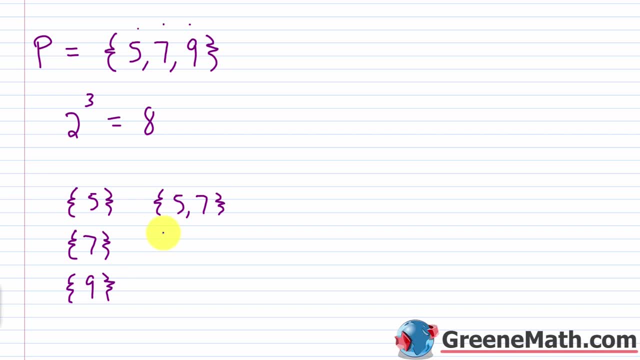 have 5 and 7.. Another would be 5 and 9.. And another would be 7 and 9.. Then another one would contain all of the elements. And what is the last one? A lot of people don't get this And it's something you kind. 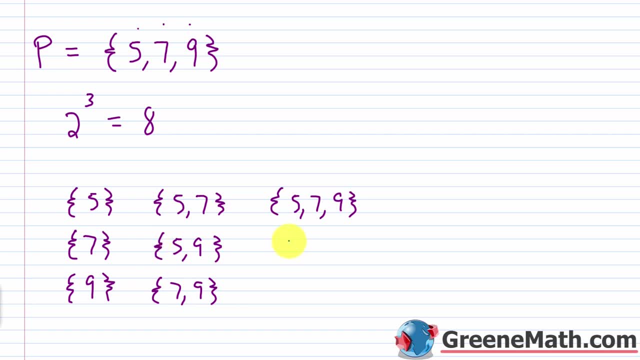 of need to be told. Well, the empty set is considered to be a subset of all sets, And why is that the case? That's one thing that many students struggle with. Well, you have to think of subsets as possible choices from the set, So I can choose 5.. I have that. I. 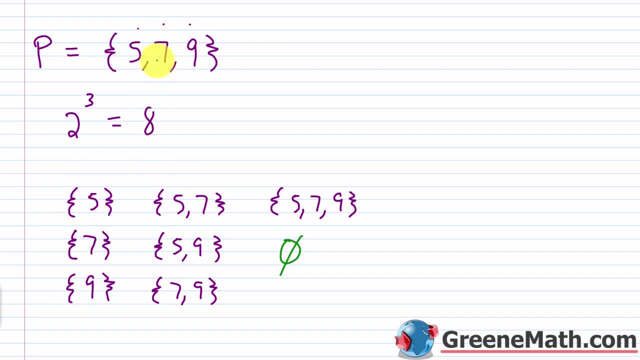 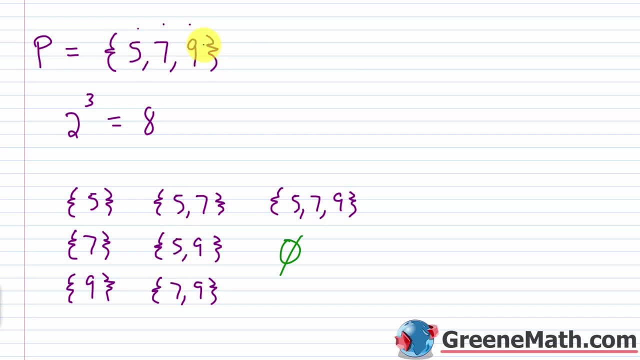 5 and 9.. I can choose 7 and 9.. I can choose 5,, 7, and 9.. Or I can choose nothing. I can choose nothing. So as an example we can kind of understand, Let's say that I have a set L, So I have a. 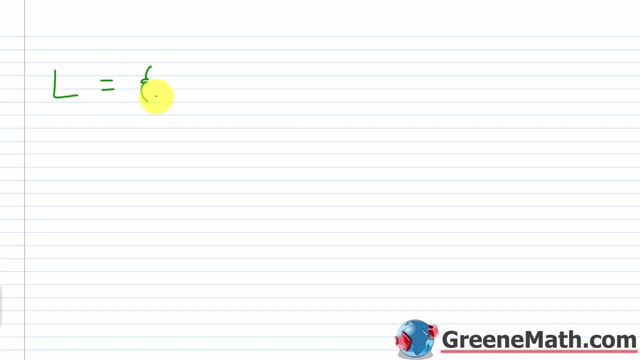 set L, And L contains three elements. It's the elements that are in my lunchbox that I'm bringing to work. So let's say I have chips, I have soda and I have a sandwich. Make it real simple. So what are the possible subsets that I can make here? We know there's. 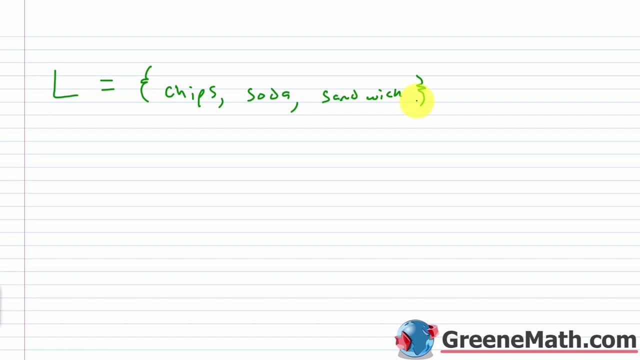 three elements so that we know there's going to be eight using our formula. But let's go ahead and list them Again. think about possible choices. What can I take out of the lunchbox? Well, I could take out just chips. I could take out just a soda. I could take out just 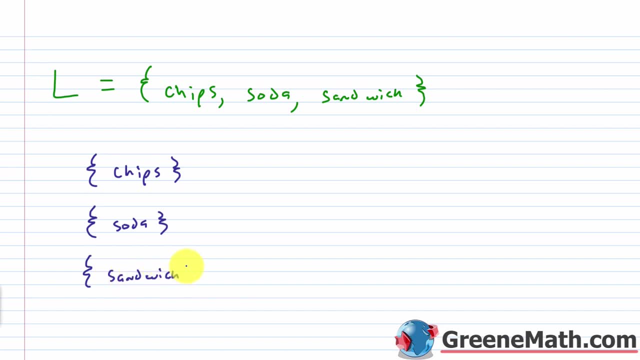 a sandwich. Now I could take out two items. if I wanted to, I could take out a sandwich. I could take out chips and soda. I could take out chips and a sandwich. I could take out a soda and a sandwich. Then I could take out all three. if I wanted to, I could take out. 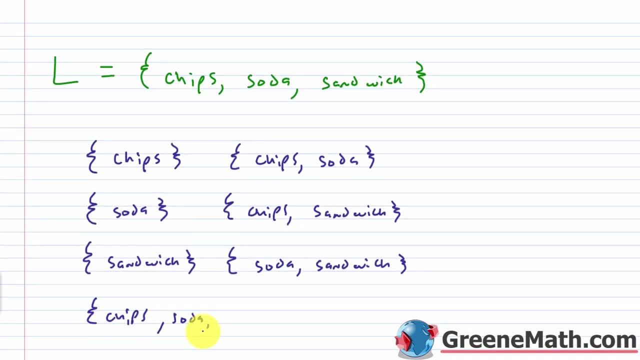 the chips, the soda and the sandwich, Okay. And then, lastly, I could choose to just take out nothing, right? I could choose to open my lunchbox up and say you know what? I don't want anything. So my choice is to choose nothing. 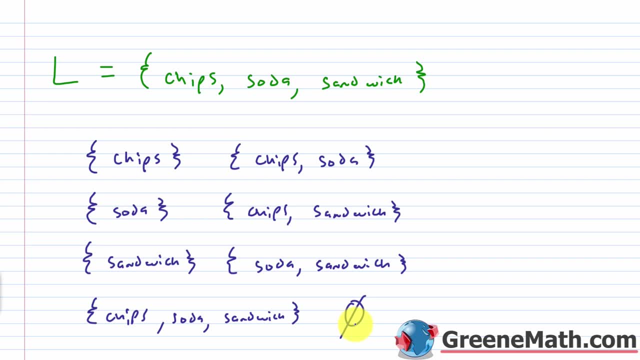 So that becomes the empty set choice, And so I have my subsets. I have one, two, three, four, five, six, seven, eight, And that is given to me by my formula, which is two raised to the number of elements I have. I'm going to have one, two, three elements, Two to the. 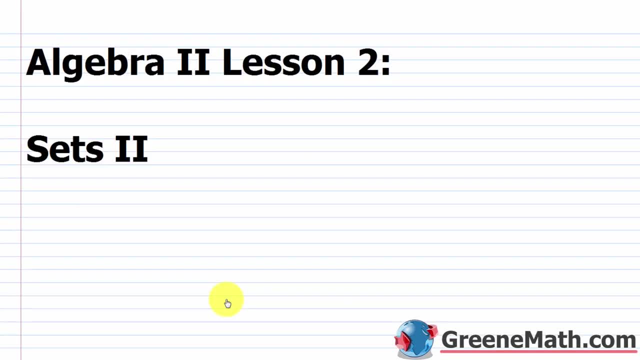 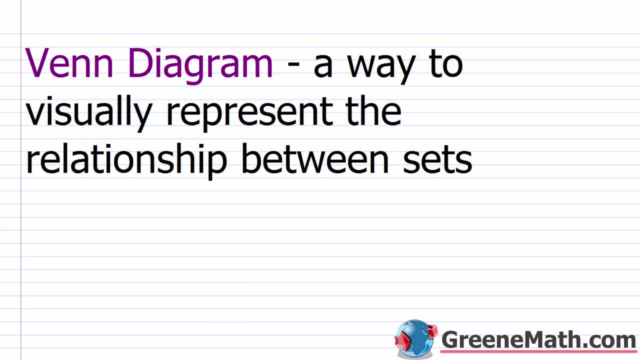 third power is eight, And I've listed them there. Hello and welcome to Algebra 2, Lesson 2.. In this video we're going to continue to learn about sets, So at some point in your math class you've probably heard about something. 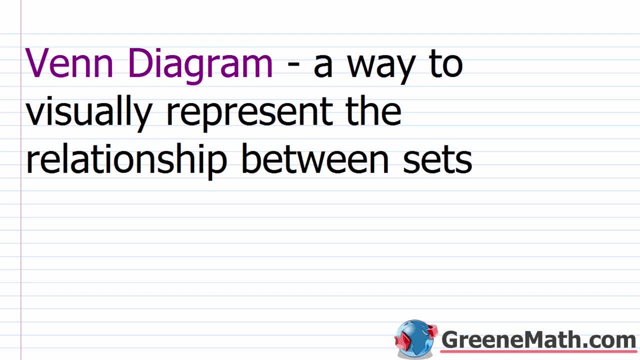 known as a Venn diagram. If you haven't, I can promise you by the time you get out of high school you're going to encounter at some point, either in a math class or outside of a math class. But a Venn diagram is just a way to visually represent the relationship. 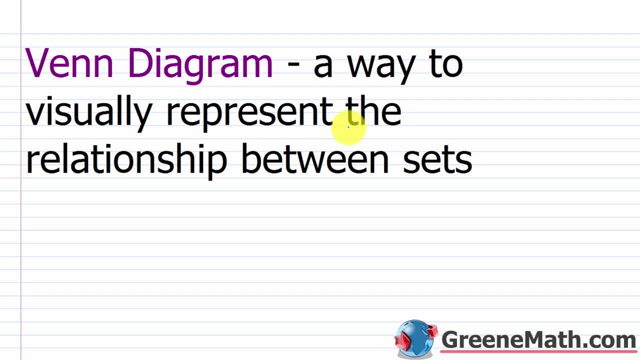 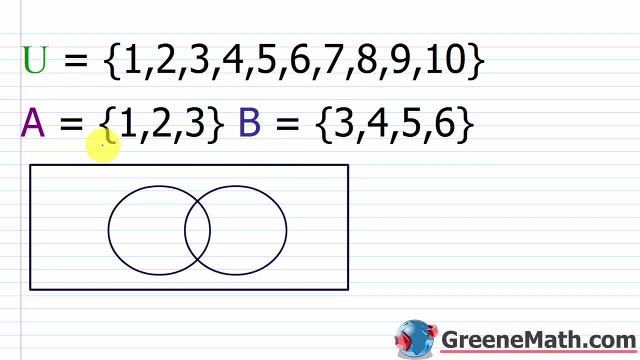 between sets. It's actually a very, very useful thing, even when you're not working with math. So, as an example, let's say we have a universal set which contains the elements one through ten. Then we have a set A, which contains the elements one through three and a set. 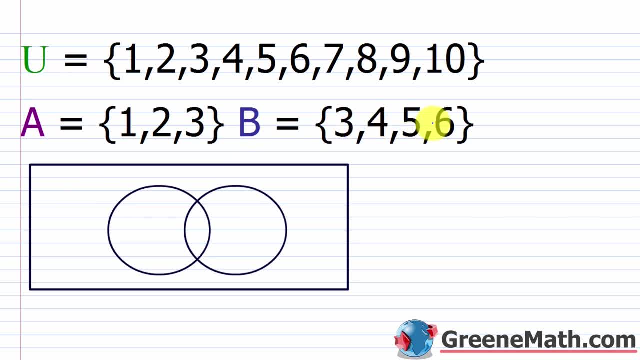 B, which contains the elements three through six. So the idea here is that we draw a rectangle to represent the universe or the universal set. So let me just put a U inside of here to say this whole thing: A represents set U. So all of my elements here should be listed inside the rectangle. 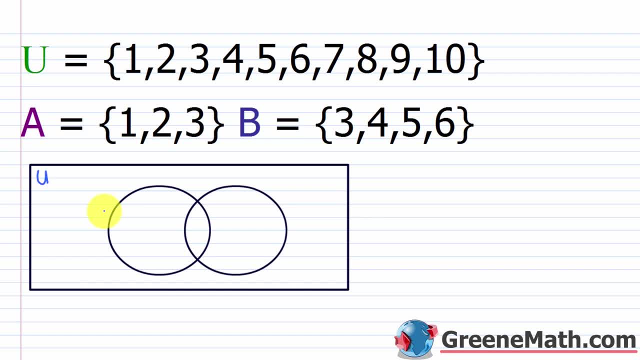 somewhere. Now I have two subsets of U, I have A, which is a subset of U, and I have B, which is a subset of U, And each of these is represented with a circle. And notice how the circles are inside of the rectangle, right inside of our universe, So I can label each. 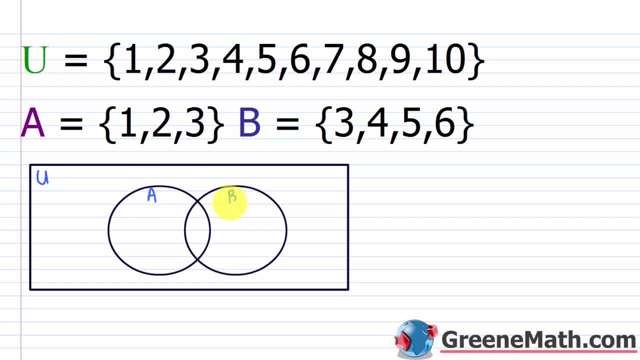 circle. I can label one of them as A and the other as B. It doesn't matter which is which, But I would list elements inside of the area that it corresponds to. And one thing I want to bring your attention to right away: I want you to notice how there's a section of overlap. 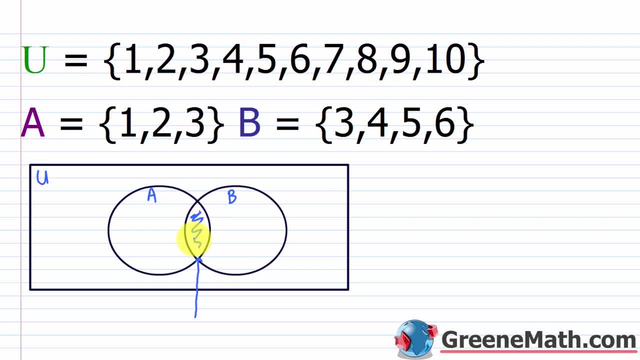 This is used to place any element that is part of set A, that is also part of set B, so a common element. And when we start listing things here, we see we have one, two and three for set A and we have three, four, five and six for set B. Three is common to. 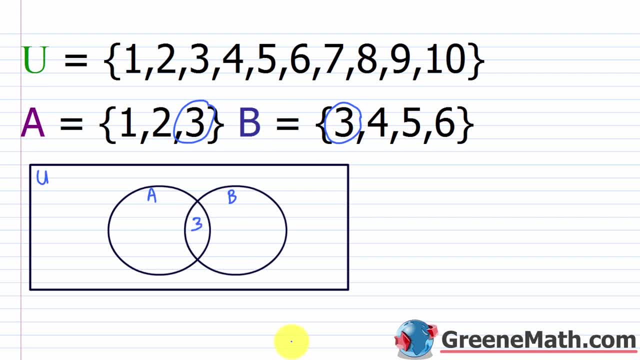 each. So that's going to go in this section of overlap. Now for set A. I have one and two that are not common to B, so that's just going to go over here somewhere outside of the overlap. Same thing goes for set B. I'm going to put four, five and six in here, but outside of 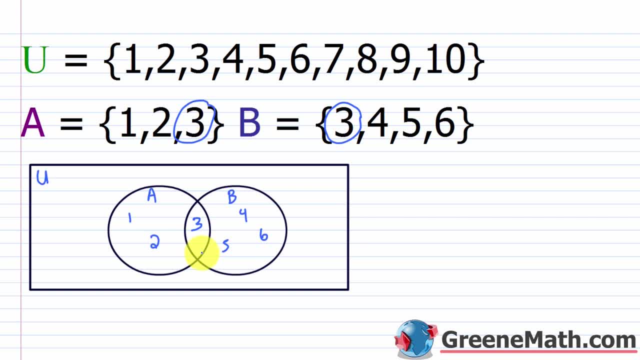 the overlap. Now, elements that are part of the universal sets, that are not part of A and not part of B, would just go somewhere inside of this rectangle. They just can't go inside of these two circles because, again, they're not part of A or B. 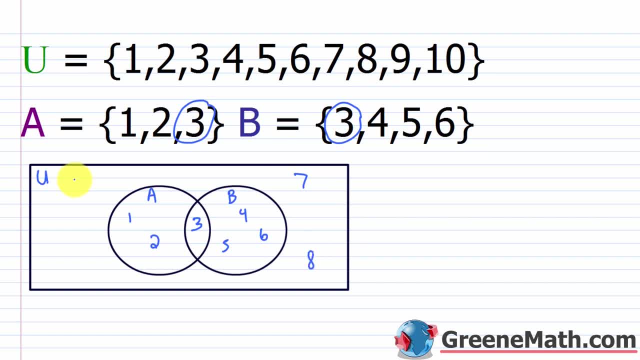 So I have seven, I have eight, I have nine and I have ten that fit that criteria. So this is our first Venn diagram. Let's just go ahead and label it. This is our Venn diagram And again, it's a visual way to represent the relationship between the sets. I can look. 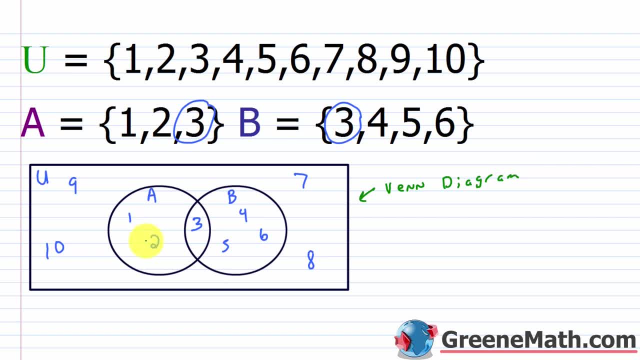 at this right away, and I can tell that I have a universal set that's one through ten. I have a set A that's one, two and three. I have a set B that's three, four, five and six, And I can also tell that A and B have a common element of three. So some key information. 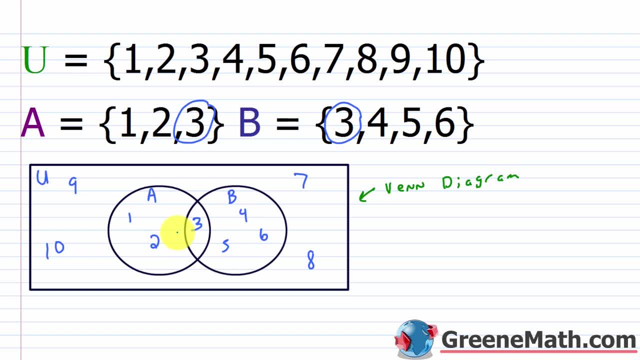 that I can pull right away just by looking at a picture, versus kind of looking at these sets in the roster method and trying to kind of pull information out that way. Now a couple of things we want to talk about now. The first thing would be the complement. 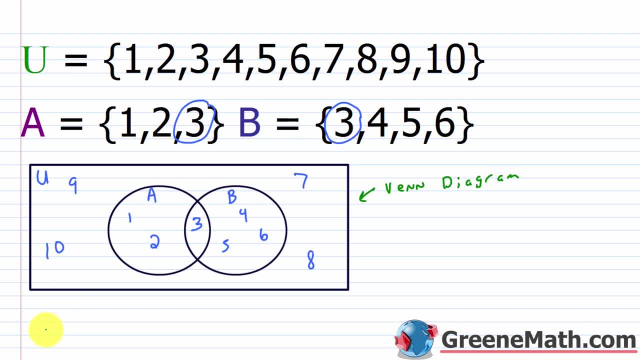 of a set. So this is represented. if I wanted the complement of A, I would write A prime or A complement like that, with a superscript C on top of the A. So A complement contains all of the elements or members of set U that are not elements or members of set A. So in 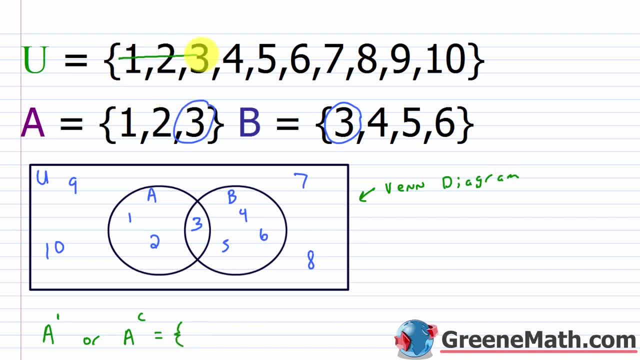 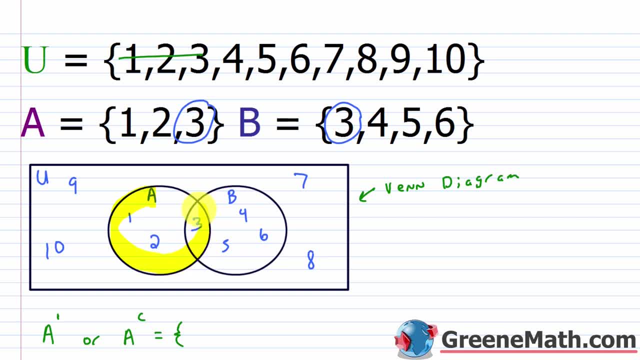 see that if this is set A, everything inside this circle- and I know I didn't color in the lines perfectly, but just you know, kind of bear with me- everything outside of that circle is the complement of A, So it's very quickly to get that. I can just see that it's. 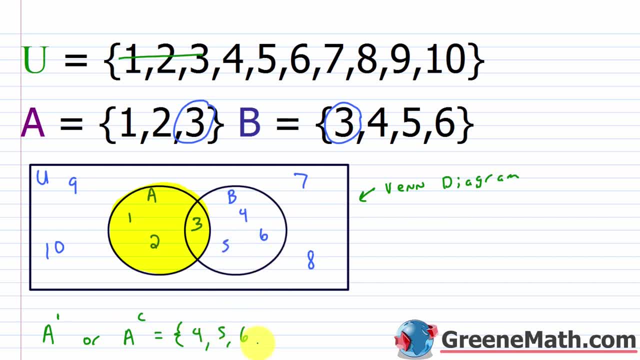 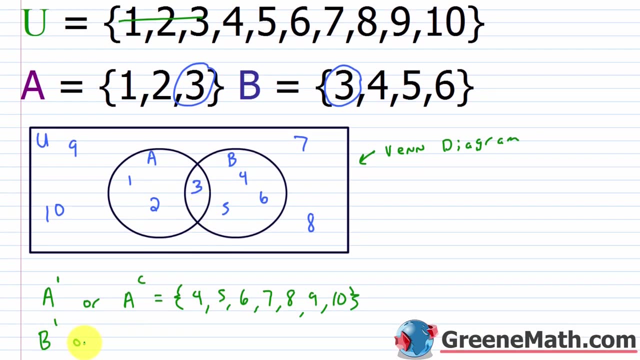 four, five, six, seven, eight, nine and ten. Very easy to get that information. As another example, let's take B complement. Let's erase this And let's take. you can put B prime or B complement like this And: 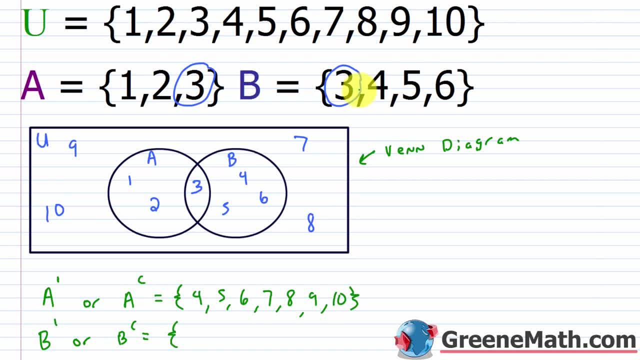 in this scenario I could either do it this way. I could say, okay, this contains three, four, five and six. I can mark those out and say it's one, two, seven, eight, nine and ten. Or visually, I could look at my Venn diagram and if I look at B, right here everything. 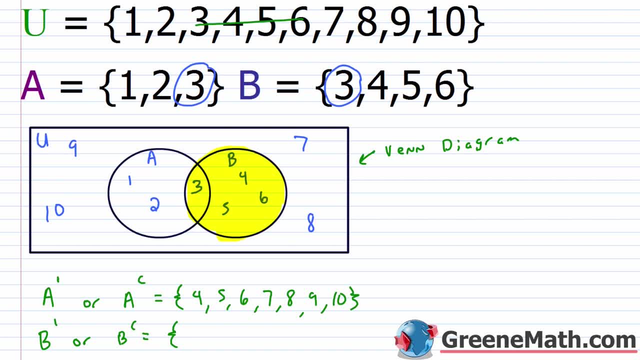 outside of this is going to be the complement of B, So I'm looking at again one, two. I have seven, eight, nine and ten, Seven, eight, eigh and ten. Now let's erase this. 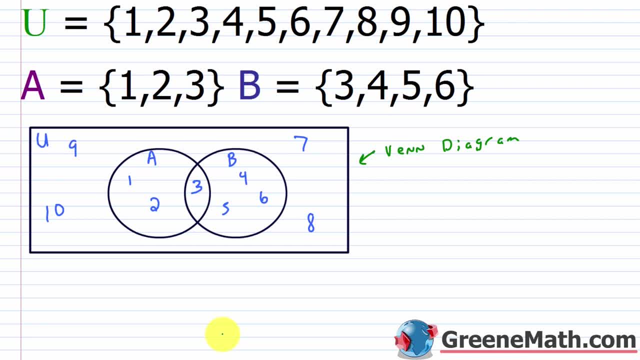 real quick. Let's now talk about the union of two sets. So the union of two sets- let's say A and B- is denoted with a symbol that kind of looks like a- U. So let's say A, let me do it in a different color union, and then that's not gonna matter. so you're gonna. just go ahead and paste that, Okay, and then you're gonna input that, And then I'll do it two times right now and then I'll save this. So I think I did that a lot. That's quite an. 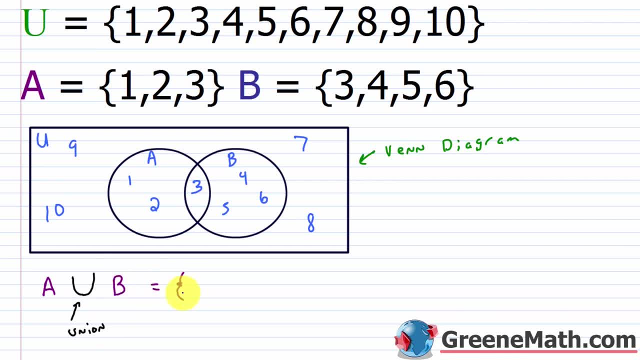 let's return to the other color. b is equal to. this is going to be the set of all elements of a, along with all elements of b, but with one key thing here. we don't want to double list anything, okay? so if i put in all the elements from set a, that's one, two and three, then all the elements. 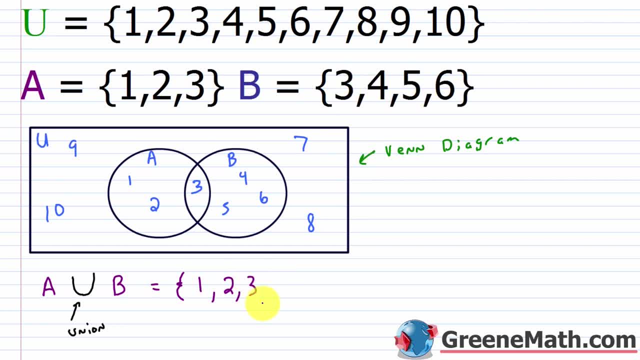 from set b. i've already listed three, i don't need to list it again. so then just four, five and six, and again the way you look at the union is: if i look at my venn diagram, it's everything that's contained in these two circles. so everything in these two circles. what's not going to go in there? 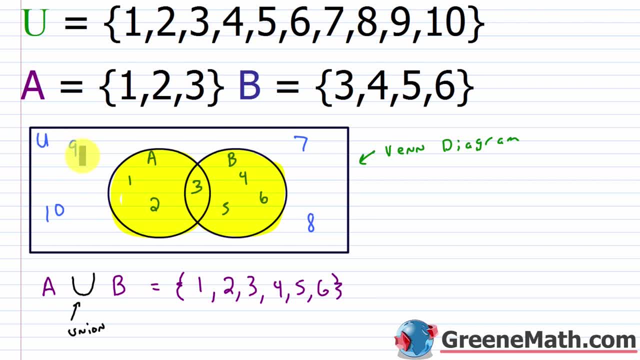 would be anything outside of the circle. so things like eight, seven, nine and ten, things that are outside of the circles. you can very quickly look at the venn diagram and get the union now. the other thing that we would talk about would be the intersection. so let me erase this real quick. 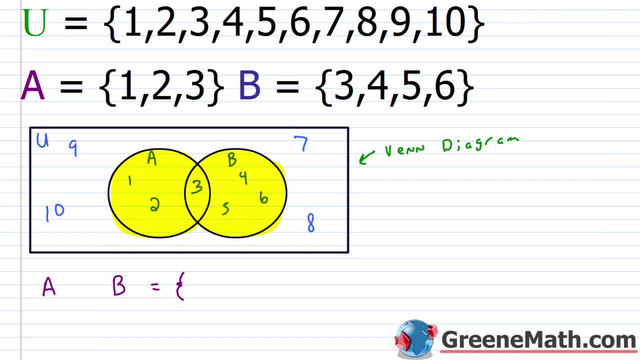 the intersection just looks like a flipped upside down u, so i'm just going to basically reverse that symbol and make it look like this. so this is intersection, and the intersection of a and b is going to be the set of all elements that belong to both a and b, and again, that's where you're going to look at your overlap. so if i look at 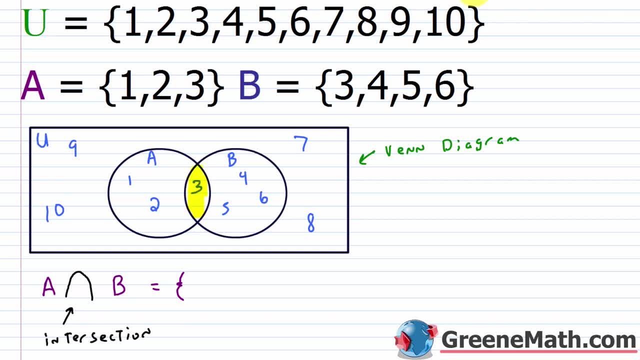 my venn diagram. this is the intersection, again the set of elements that belong to both a and b. so that's going to have one element. so a intersect b is equal to: we just have one element and that element is three. all right, let's take a look at another example. so here we have a universal set where we have: 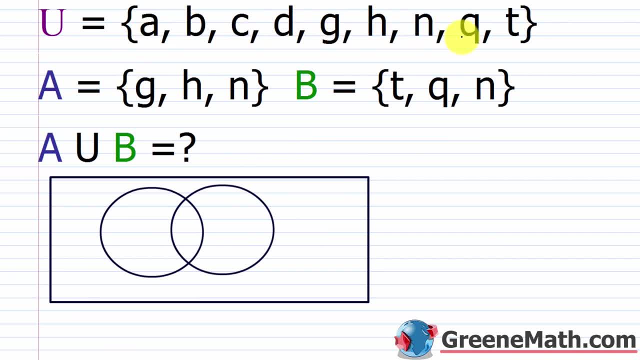 the elements a, b, c, d, g, h, n, q and t, and everything is in lowercase to keep you from confusing it with the set names. then we have set a and capital a, and this contains the elements g, h and n, and then set b, which contains the elements t, q and n. so the first question i have here is: what is? 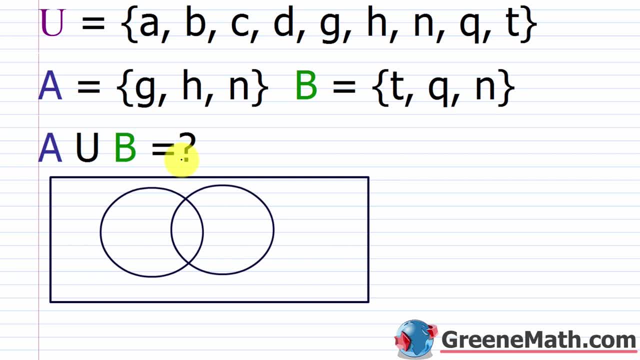 the union between a and b. so a union b equals what? well, let's fill in our venn diagram. so let's let this be set a, let's let this be set b. and in set a i have g, i have h and i. and notice where I put the N: It's because it's common to A and B. 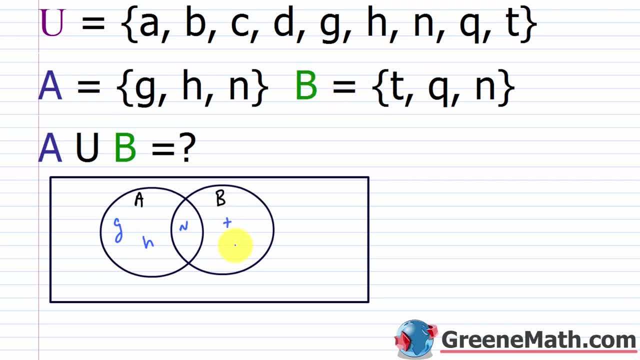 So for set B I have T, I have Q and again I have N. N is in the overlap section because it's a member of set A and also set B. Now in my universal set I have elements that are not part of A and B. I know that A falls outside of. 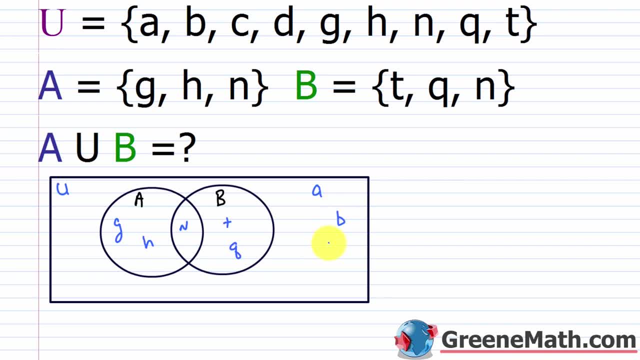 those two circles. so does B, so does C, so does D, G doesn't, H doesn't, N doesn't, Q doesn't and T doesn't. So if I want the union of A and B, this is going to be equal to. 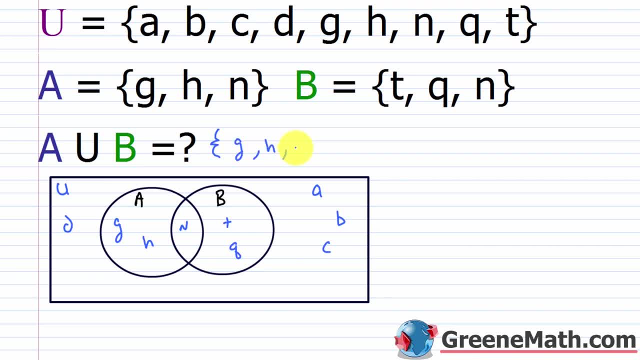 we'll have G, H, N, T and then Q And again, the main thing here is to make sure you don't double list anything. So I have N here and here. it only gets listed once when I fill out this information. What if I ask for the intersection? 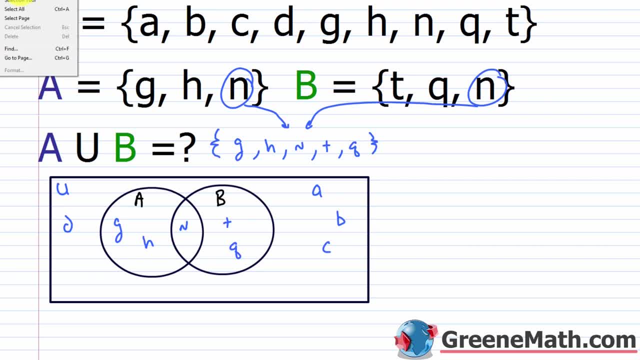 If I said, let me kind of go in here and edit. So if I ask for the intersection, the symbol looks like this: Just an upside down U, and I know that's not perfect but just pretend it is. Again, I'm looking for the overlap between these two sets. So the overlap, if I 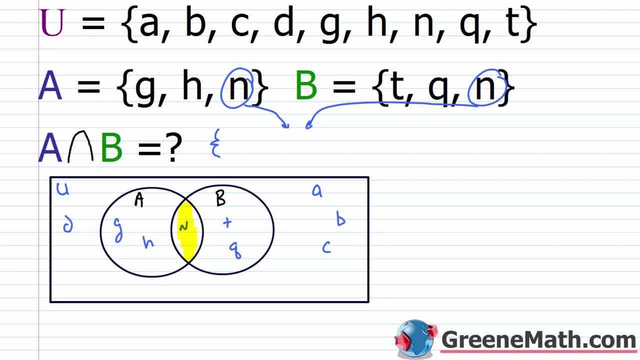 look at the Venn diagram. it's just going to be right here. That's real easy to get. That's N. So that's A intersect B. And then what if I ask for some other things? Let's say I asked for A complement. 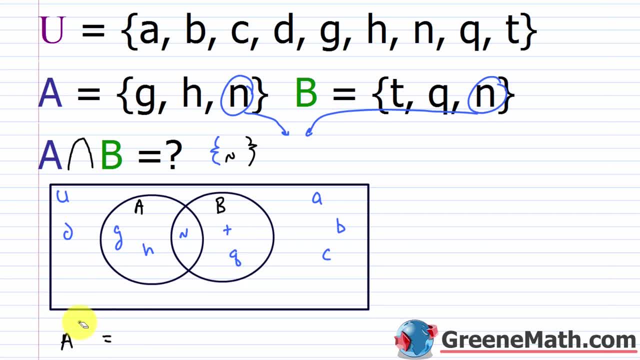 A complement, And I could do it this way, or again I could do it this way, doesn't matter. Well, that's anything that's outside of A. So I could just highlight this set right here and I could look for things that are outside of A, and what I'd come up with is: 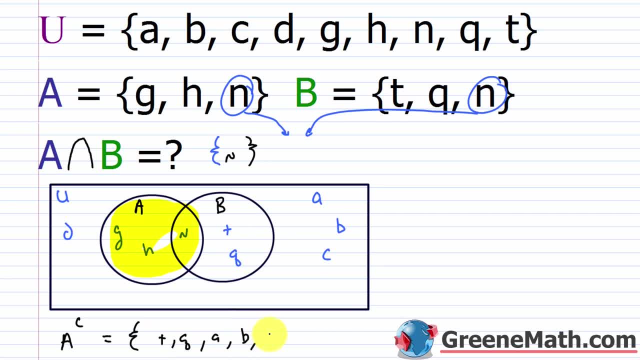 T, Q, A, B, C and then D, And again, it doesn't have to be in alphabetical order. The order is irrelevant when you're listing the elements of a set, And if I ask for B complement, that would be anything, that's. 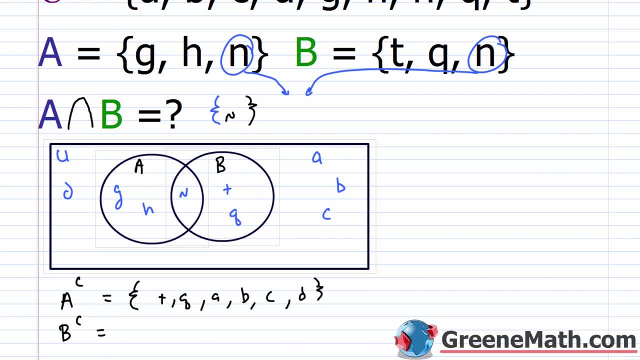 outside of this circle here. So let me highlight that real quick for you. So for this case, I'm looking at what I'm looking at A, B, C, G, H and D. Alright, let's take a look. 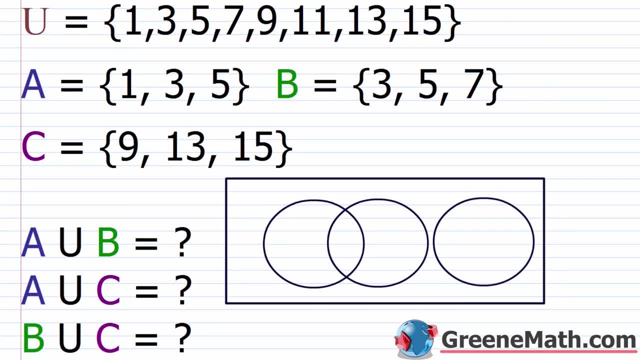 at another one. So now we're going to have our universal set, which contains 1,, 3,, 5,, 7,, 9,, 11,, 13, and 15.. So basically the odd numbers, starting at 1 and going through and including 15.. Then set A: 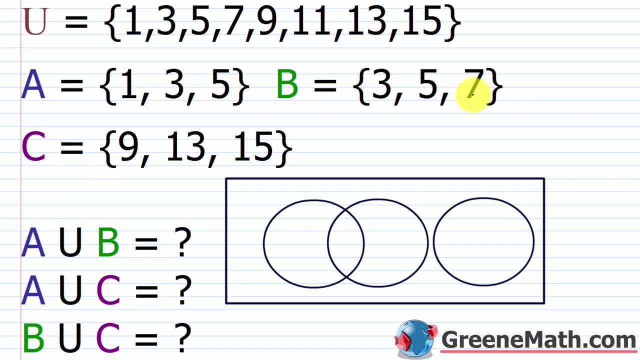 has 1,, 3, and 5.. Set B has 3,, 5, and 7.. And set C has 9,, 13, and 15.. So let's label this as set U. Let's label this as set A. 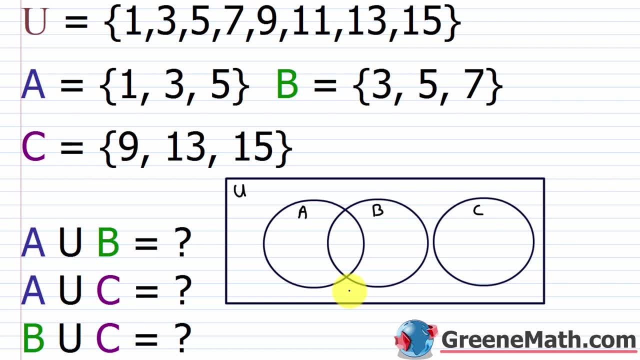 set B and set C. So now what you're going to notice is set A and B have 2 common elements, 3 and 5. So those are going to be put in the overlap section And then for set A we have 1, that's. 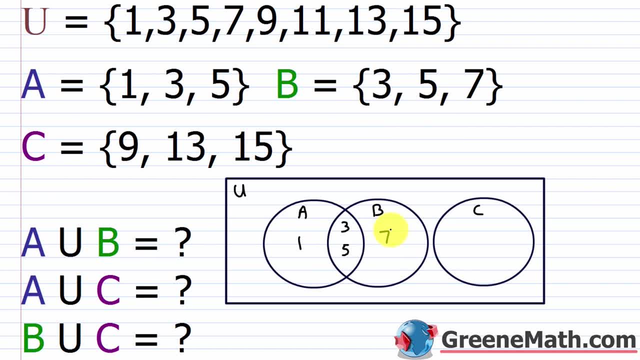 outside of that, For set B we have 7. that's outside of that. And then for set C we have nothing that's common to A and B. So notice how there's a gap between these circles. We don't want any overlap because there's nothing that's going to be. 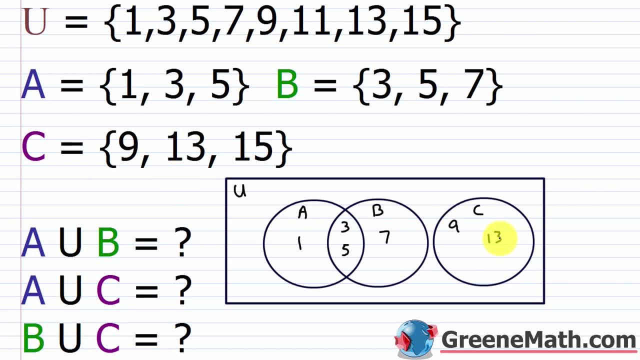 common. So for set C I'm going to write in 9,, 13, and 15.. Okay, so also in set U we have 11. that's not listed in any of these sets here, So that's going to go outside of all those. 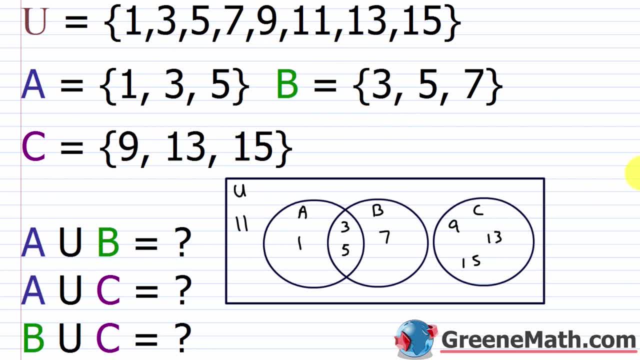 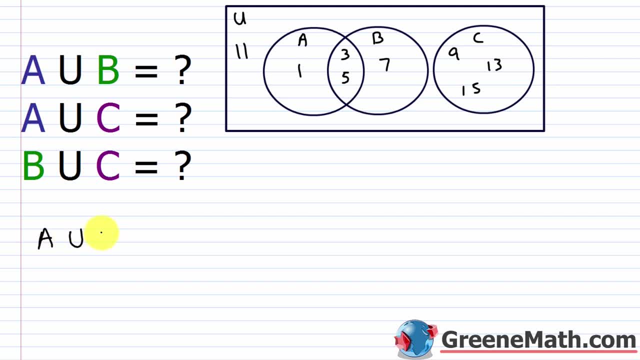 circles. So, without referencing to this, let's answer these questions here. So we're just going to look at our Venn diagram. So we have A union B, What is that? That's all the elements of A along with all the elements of B. Again, just don't double list anything. So, looking at the Venn, 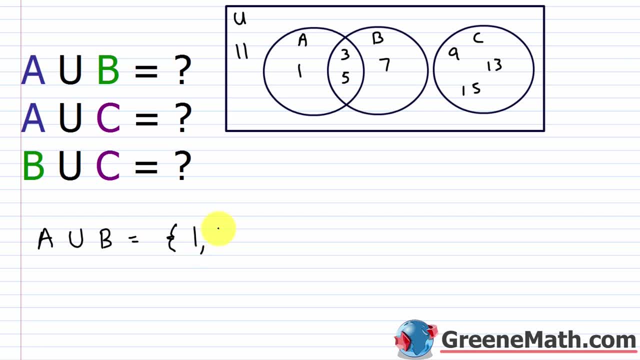 diagram. that's easy. It's a 1,, a 3,, a 5, and a 7.. Then, if I want A union C, what is that? Well, that's 1,, 3,, 5,, and then 9,, 13,, 15.. 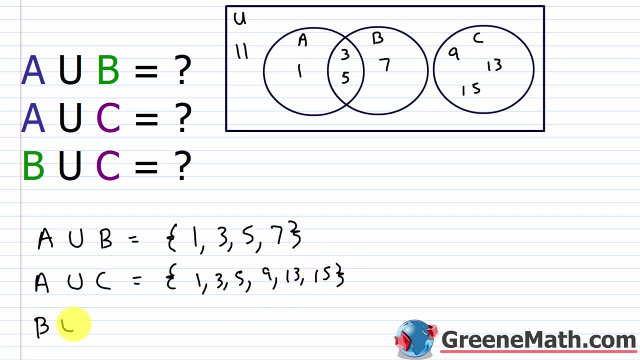 And then B union. C is what We have: 3,, 5,, 7, and then 9,, 13,, 15.. Let's see if we can do some other things here. Let's erase this And let's ask for the. 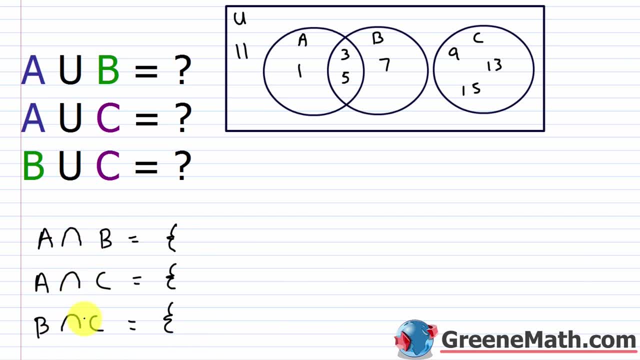 intersection in each scenario now. So A intersect B is what? Again, that's your overlap here. So that contains the elements 3 and 5.. What about A intersect with C? There is no overlap. Those two sets are called disjoint sets. They have no elements. 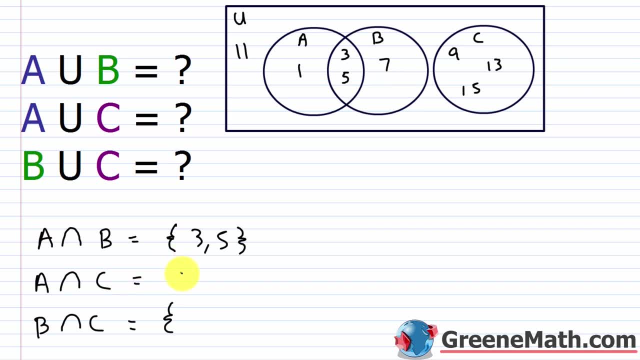 in common, And so this right here would be the null or empty set, because this set contains no elements, because there are no elements that are common between set A and set C. Same thing goes for the intersection of B and C. You would put the symbol for the null or empty set. 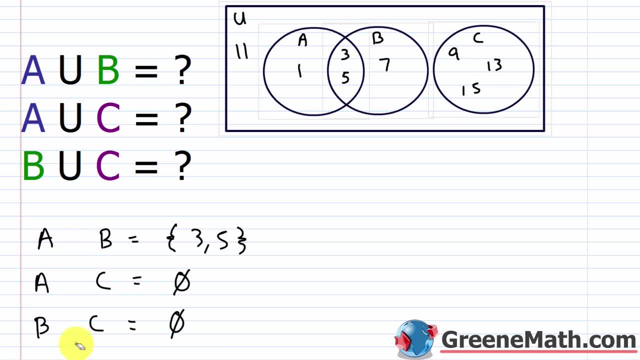 Now we could also go through and we could do the complement of each. So I could do the complement of A, the complement of B and the complement of C, And again with our Venn diagram we can do these very quickly. 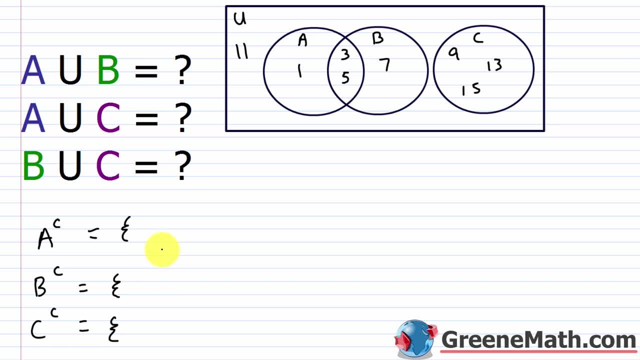 So for A complements I would have 7,, 9,, 13,, 11, and 15.. For B complements I would have 1,, 11,, 9,, 13, and 15.. And then for C. 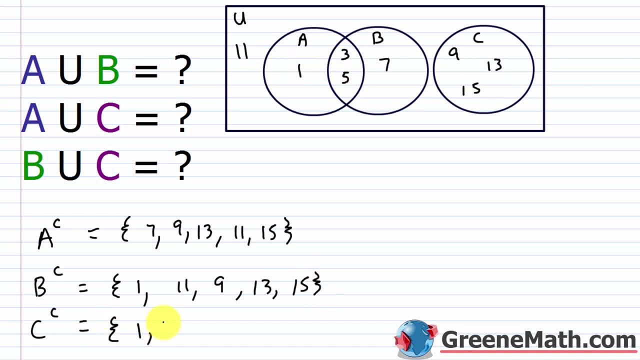 complement, I would have 1,, 3,, 5,, 7, and 11.. And again, just looking at the Venn diagram makes things nice and easy to see. If I want A complement, I could shade A and say I want everything outside of that. so that's. 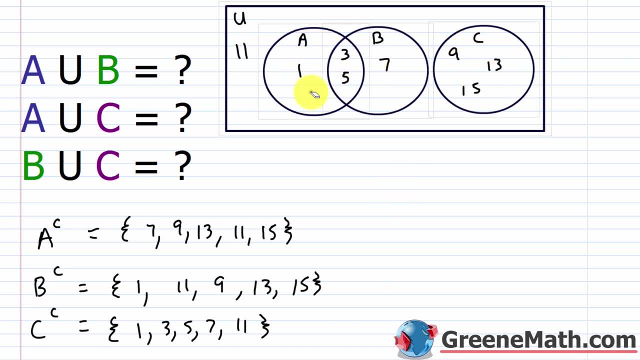 7,, 11,, 9,, 13, and 15.. If I want B complement, shade B, and I want everything outside of that. so that's 1,, 11,, 9,, 13, and 15.. And if I want C complement, I could shade. 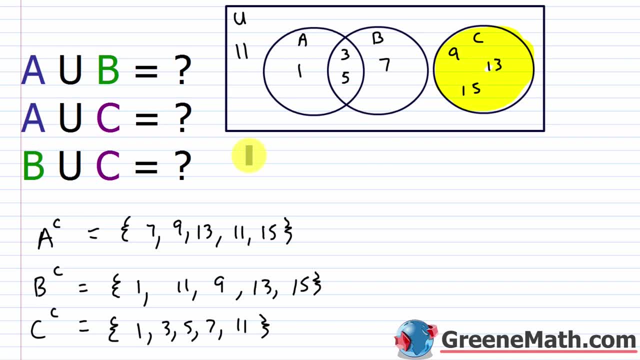 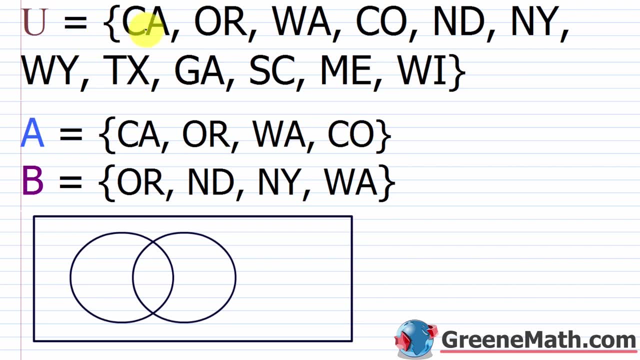 C and again, I want everything outside of that. so that's 1,, 3,, 5,, 7, and 11.. Alright, let's take a look at another one. So we have a universal set that contains California, Oregon. 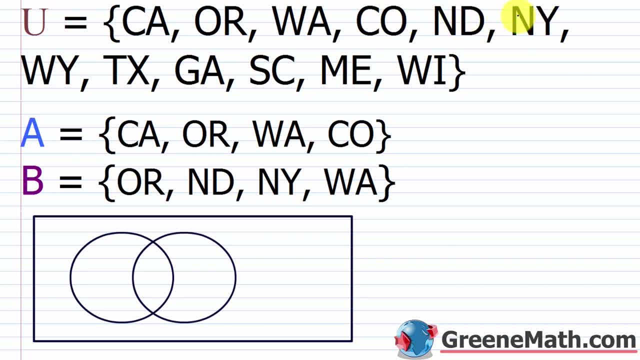 Washington, Colorado, North Dakota, New York, Wyoming, Texas, Georgia, South Carolina, Maine and Wisconsin. Then I have a set A, which is a subset of set U, which contains California, Oregon, Washington and Colorado. Then I have a set B, which again is a subset of. 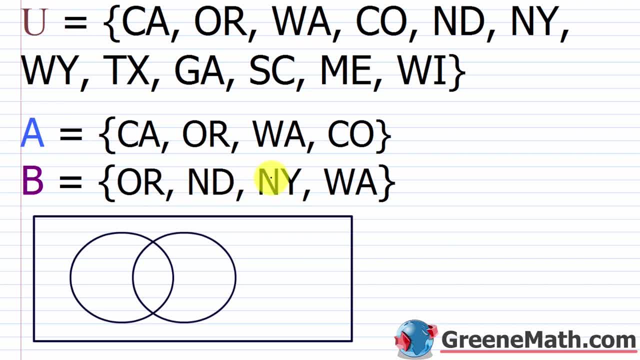 set U, which contains Oregon, North Dakota, New York and Washington. Now if I fill this out for set A and set B, what they have in common would be Washington and Oregon. So let's say this is set A and this is set B. 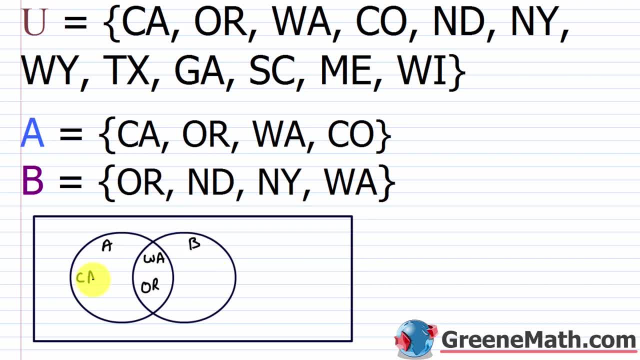 So for set A, I would also have California and I would have Colorado. For set B, I would also have North Dakota and I would have New York, And outside of these sets, in set U, let me use a different color. 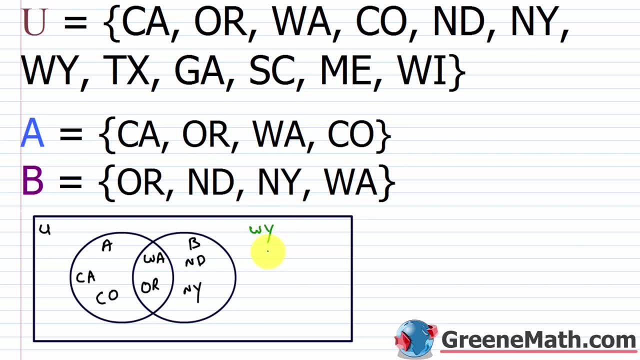 I would have Wyoming, I would have Texas, I would have Georgia, I would have South Carolina, I would have Maine and I would have Wisconsin. So once we have our Venn diagram built, it's easy to go through and answer some questions. So let's say I start out by asking you for 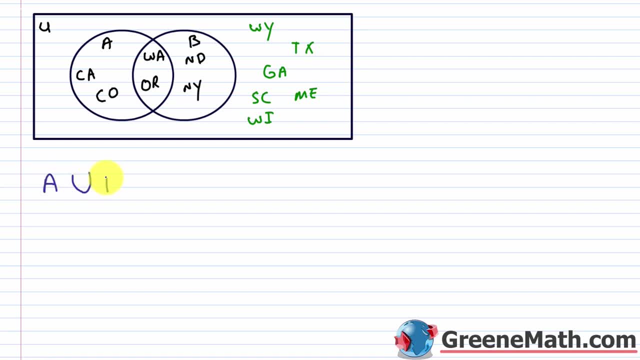 A union B. What's that? equal to Well, that would be California, Colorado, Washington, Oregon, North Dakota and New York. If I asked you for the intersection of A and B, that would be the overlap section, So that would contain two states: Washington and. 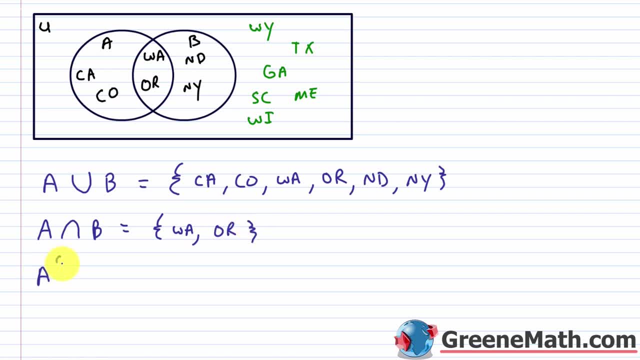 Oregon. If I asked you for A complement again, I could highlight this right here and I could say that A complement contained North Dakota, New York, Wyoming, Texas, Georgia, South Carolina, Maine and Wisconsin, And then, lastly, if I asked for B complement, this would contain 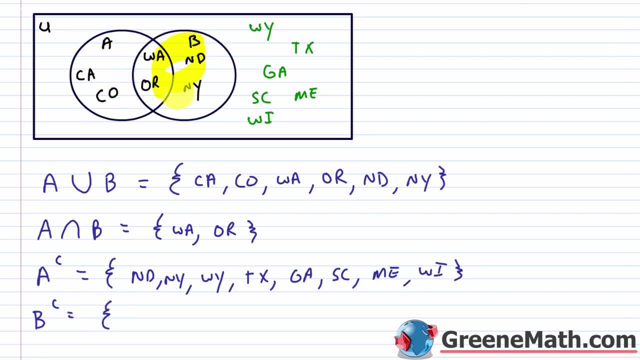 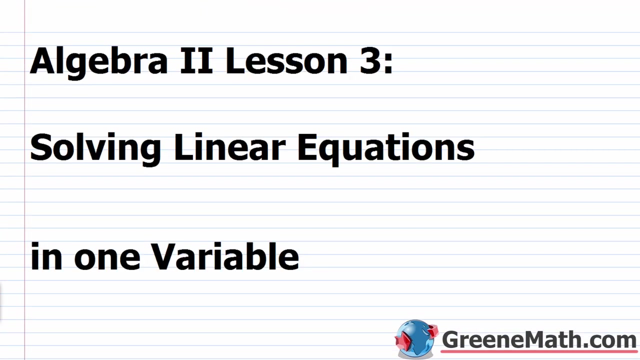 the elements. I could erase this and I could highlight this, and I could highlight this and I would have California, Colorado, Wyoming, Texas, Georgia, South Carolina, Maine and Wisconsin. Hello and welcome to Algebra 2, Lesson 3.. In this 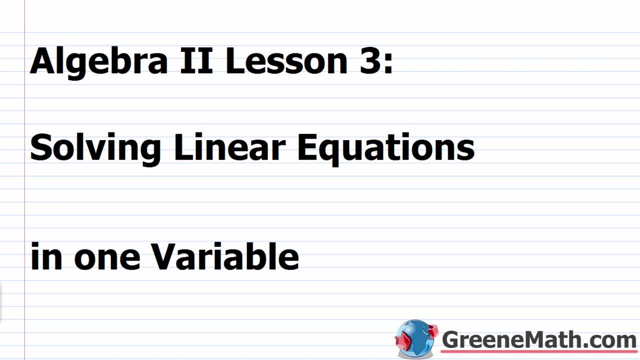 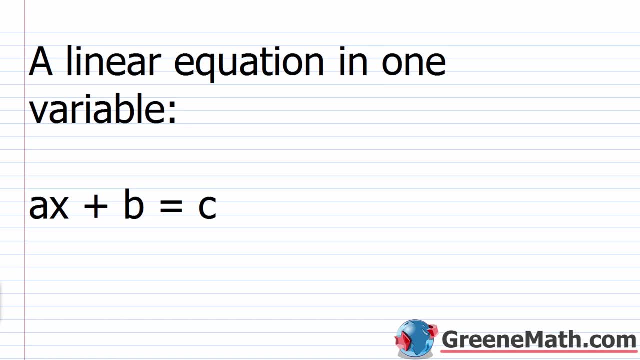 video we're going to learn about solving linear equations in one variable. So back in Algebra 1, we learned how to solve a linear equation in one variable and hopefully at this point you've completely mastered that concept. But in case you haven't, we're going to do a full 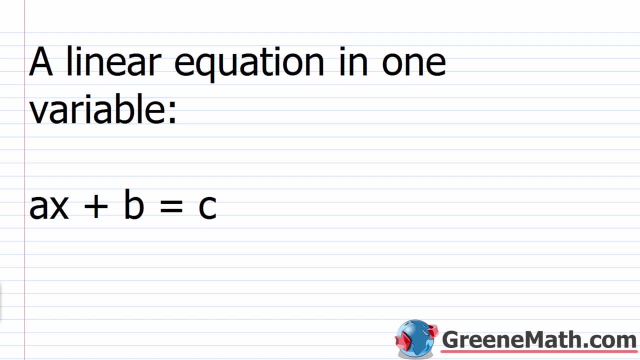 review in this video here and that's going to serve as a stepping stone for the more challenging types of equations that we're going to look at in Algebra 2.. Alright, so you will recall that a linear equation in one variable looks like this: 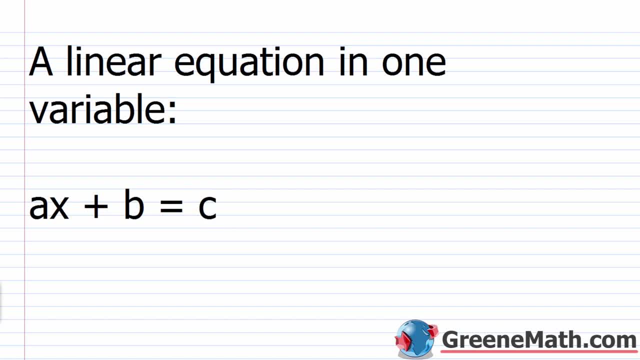 We have AX plus B equals B. So if you're in a textbook following along, you'll see something like this, And this is a generic form that you get. A, B and C are just representing real numbers. So this right here, this right. 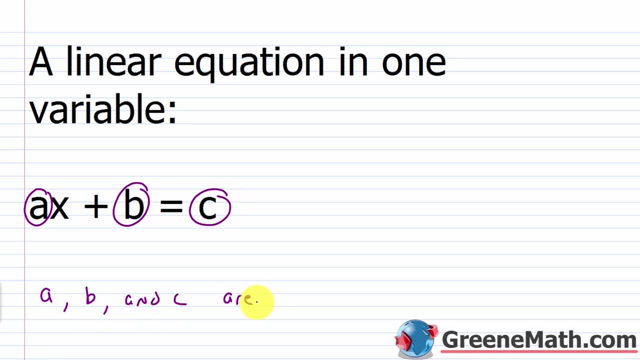 here and this right here. So we'll put: A, B and C are real numbers. And then there's one exception to this: A, which is the coefficient for X, cannot be 0. So A cannot be 0.. And obviously, 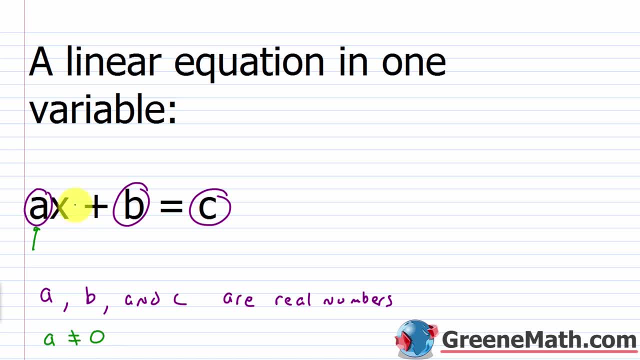 that's the case because we want our X to be there. We want our variable to be there. If I put a 0 in for A 0 times, anything is just 0. So this would disappear. We would no longer have a linear equation in one. 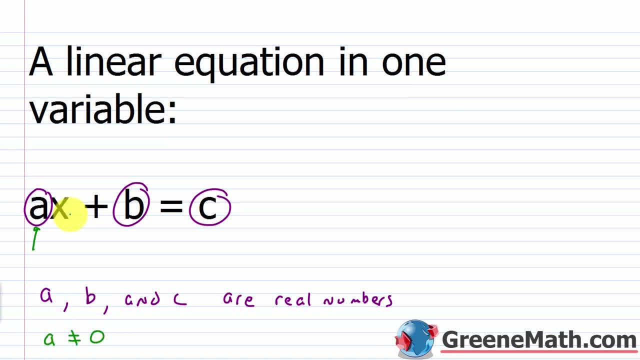 variable. So we've got to have that restriction there Now, because this type of equation contains real numbers and a single variable. in this case it's X raised to the first power. we sometimes refer to this type of equation as a first degree equation, So you might hear that in your class. 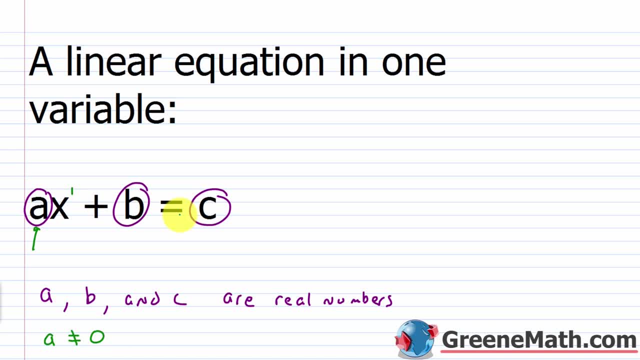 So some examples, and I know we've seen many of these. but 3X plus 5 equals 7.. So that's a linear equation in one variable, Or something like 2Z minus 5 equals, I don't know- let's say 11. Or 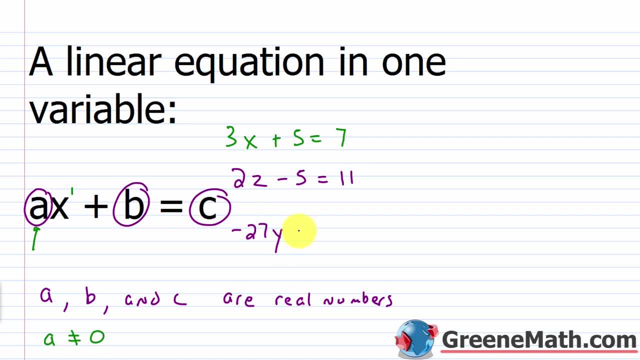 let's say negative 27Y plus square root of 2 equals negative 15.. These are each an example of a linear equation in one variable. Now, something that wouldn't be a linear equation in one variable. Let's say you had two variables involved, So something like 2X minus. 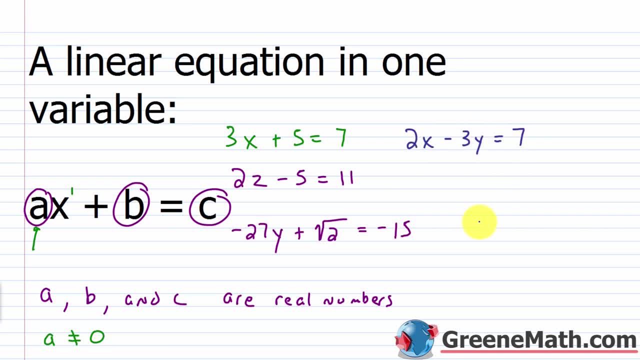 3Y equals 7. Or something with an exponent on the variable that's higher than 1.. So let's say 3X squared minus 5 equals 2.. So these two right here would not be an example of a linear equation in one variable. Alright, so let's take a look at 2X. 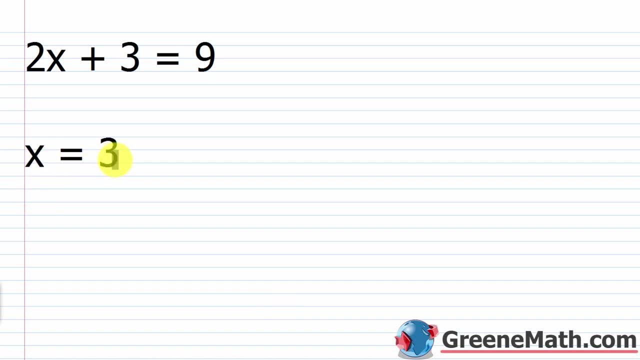 plus 3 equals 9.. And we see here that we have X equals 3.. So the first thing we're kind of taught when we start learning about equations is that the solution to an equation is a number, or it could be more than one number in some. 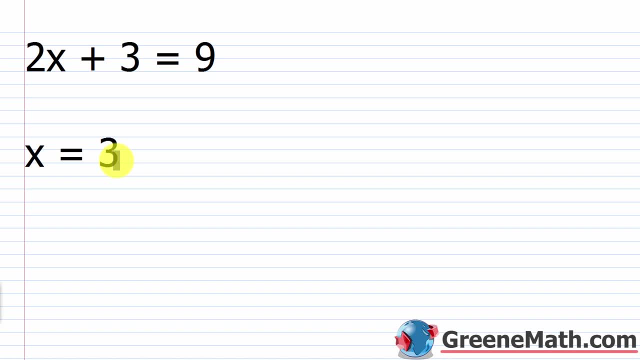 cases that when it replaces the variable- or you could have variables involved- it's going to give you a true statement. So what that means is that if X is equal to 3, if I plug a 3 in for X in this equation, 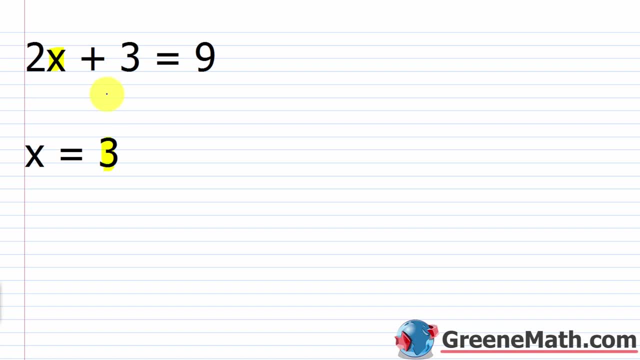 what's going to happen is the left and the right side will be the same value. So to demonstrate this, let's say I have 2 and then I substitute a 3 in for X. then plus 3 equals 9.. So over here, 2 times 3 is 6, so I'd have 6 plus 3 equals 9.. 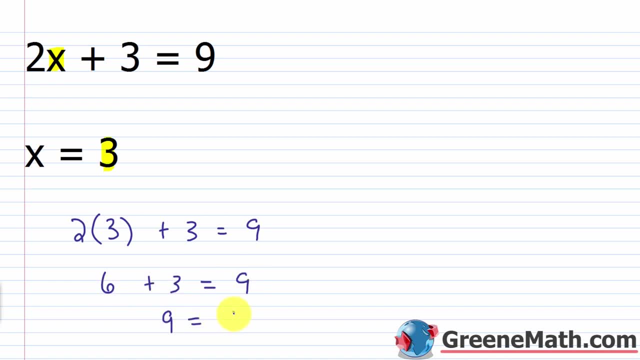 And then 6 plus 3 is 9, so you get 9 equals 9.. This is what you're looking for: The same value on the left as on the right. So that's how you know you got the right answer. Right X does equal 3 here. 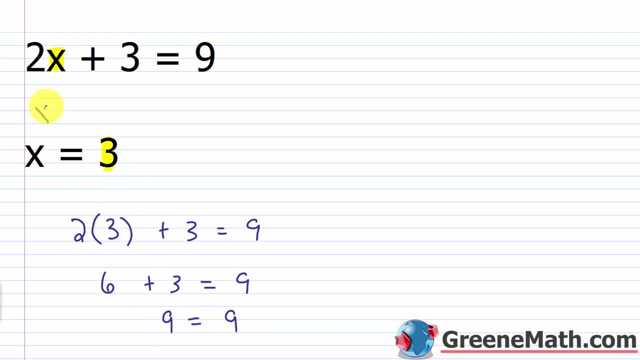 And to kind of further expand on this, let's say I chose something like X equals 4.. And I said: is that the solution? Well, I'd erase these two and say: well, 2 times 4 is 8, so I'd have 8 plus 3. 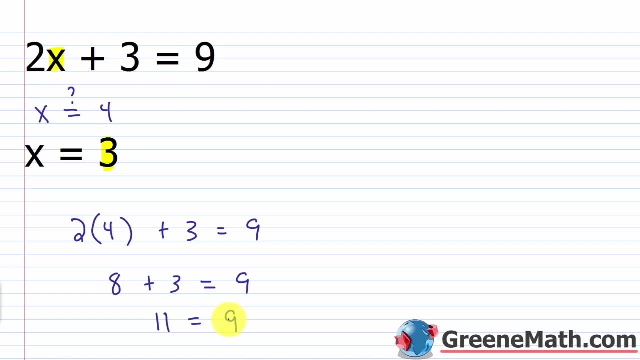 which is 11.. And no, this 11 does not equal 9.. This would be a false statement. This is false. So X does not equal 4, that's wrong. Right, we know X equals 3.. So how do we go? 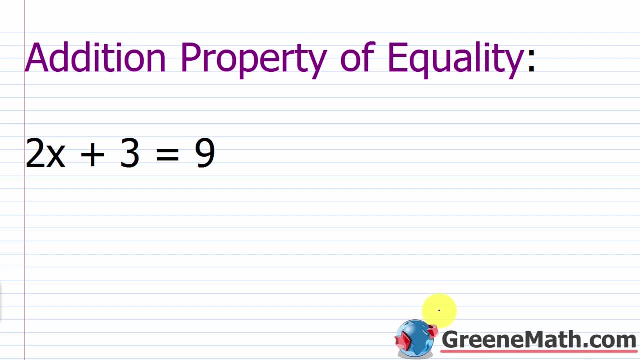 about solving a linear equation in one variable. You're not always going to be presented with the answer and just say, hey, plug this in and see if it works. So we use two properties when we first start solving equations. The first one is the addition property of equality. It tells us we can add. 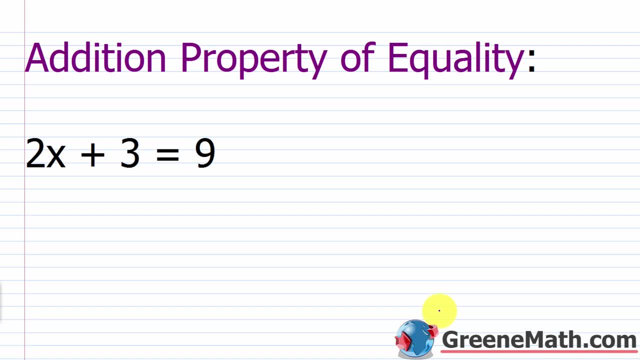 the same value to both sides of an equation and we will not affect the solution. So if I have something like 2X plus 3 equals 9, we just saw that, we know the solution is X equals 3.. Okay, we know that. Let's say I was to. 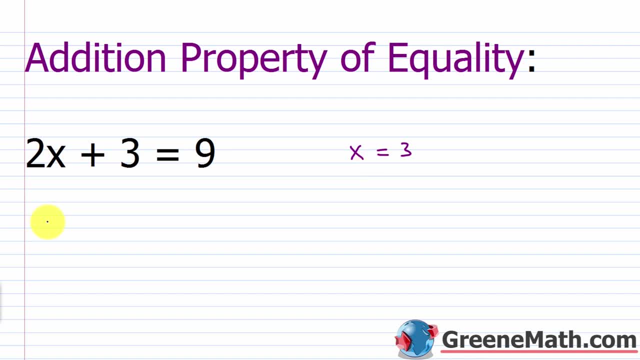 add negative 4 to both sides of the equation. So let's say we do 2X plus 3, and I'm going to add negative 4 over here, And I'm going to add negative 4 over here, And so what's going to happen is 3 plus negative 4 is what That's. 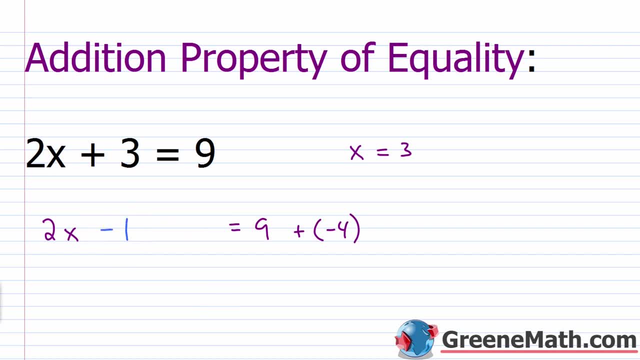 negative 1.. So I have 2X minus 1 over here, And then 9 plus negative 4 is 5.. This equals 5.. So now, if I plug a 3 in for X, will I still get a true statement? Some of you might think that you won't, but you will. 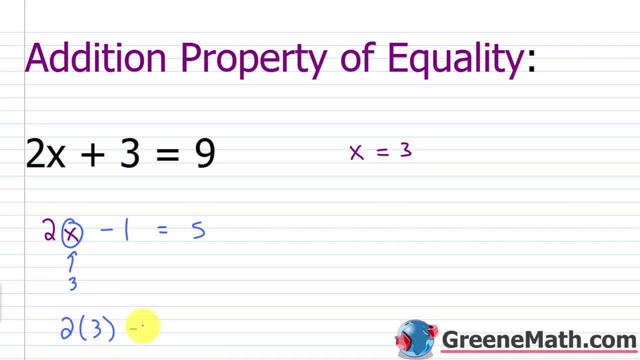 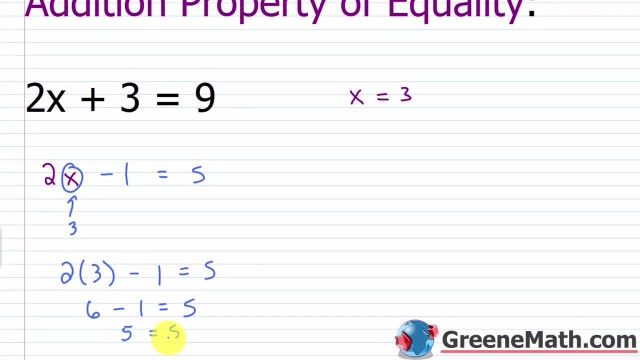 If I plug a 3 in there, I'd have 2 times 3 minus 1 equals 5.. We know this would be 6 minus 1 equals 5, and you get 5 equals 5.. So I added the same. 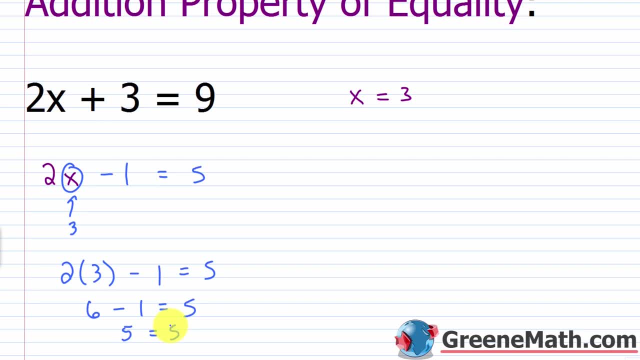 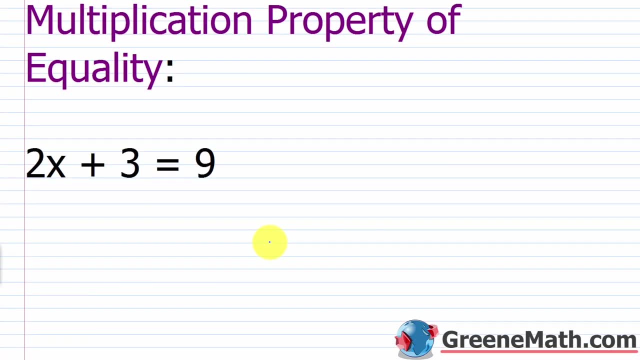 value to each side of the equation and it did not affect my solution. My solution was X equals 3 before and it's X equals 3 afterwards. Now, the other property we want to know right away is the multiplication property of equality. Now, you'll recall that. 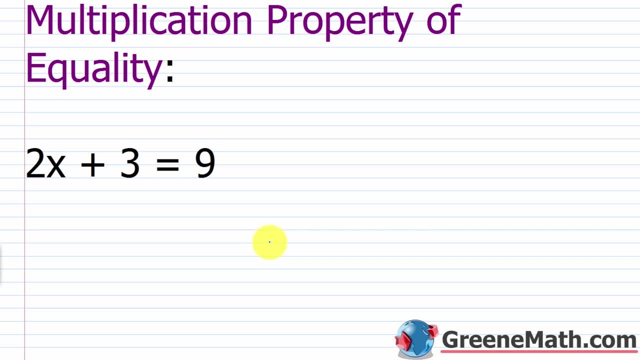 this property tells us that we can multiply both sides of an equation by the same non-zero number and it will not affect the solution. Okay, and remember you: multiply by 0, it becomes 0. So that you can't use. 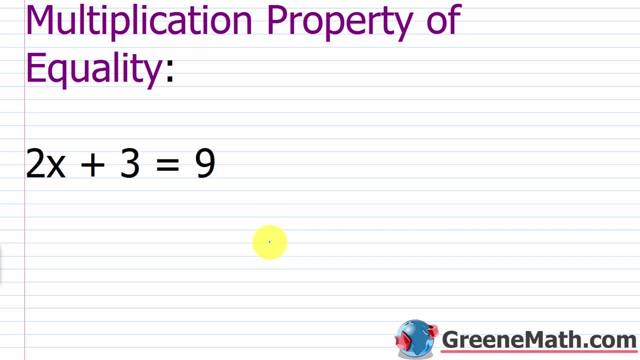 0. in this It has to be a non-zero value. So, for example, 2X plus 3 equals 9.. We know this equation has a solution of X equals 3.. If I multiply both sides of the equation by negative 2,. 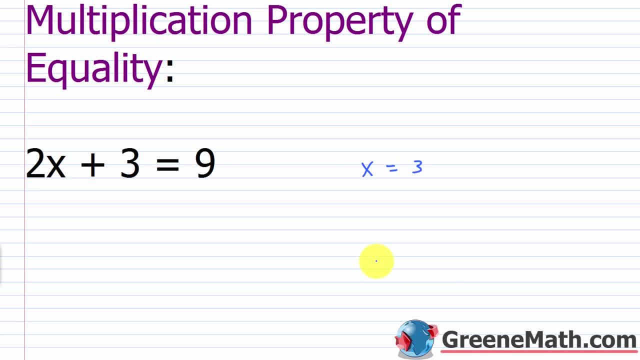 would I still have X equals 3 as the solution. Let's try it out. So 2X plus 3, let's use parentheses here. Multiply negative 2 by this side. Let's multiply negative 2 by this side. Scroll down, get a little room going. Use my. 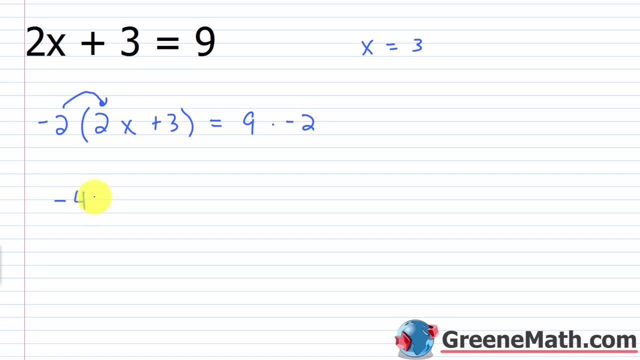 distributive property. Negative 2 times 2X is negative. 4X And then negative 2 times 3 is going to be minus 6. And this equals 9 times negative. 2 is negative 18.. Now, if I plug in a 3, 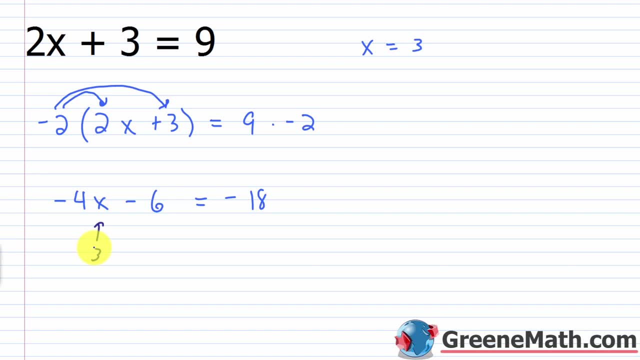 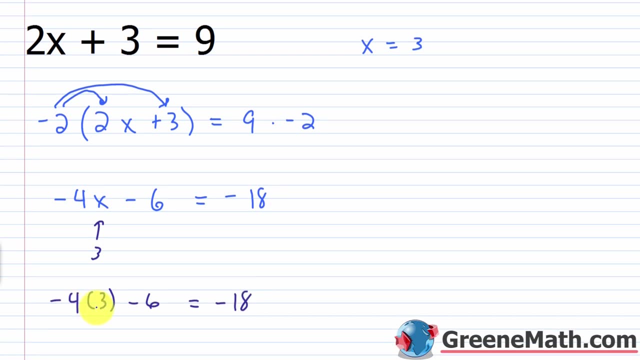 for X. am I going to get a true state? Let's see: Negative 4 times 3 minus 6 is equal to negative 18.. Negative 4 times 3 is negative 12.. So you'd have: negative 12 minus 6 equals negative 18.. And scroll down. 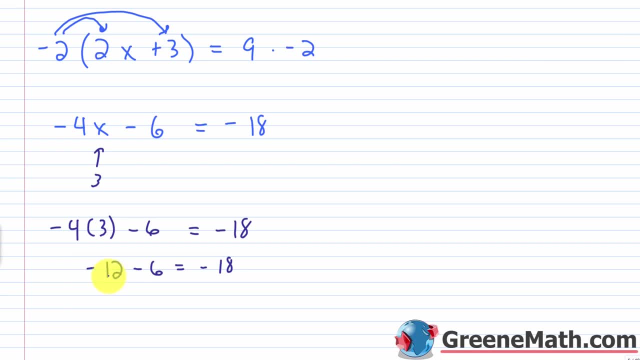 just a little bit more And what we're going to have is that negative 12 minus 6 is negative 18.. So you get negative 18 equals negative 18.. So you can see that before we multiplied both sides of the equation by negative 2, the solution was X equals 3.. After we multiplied 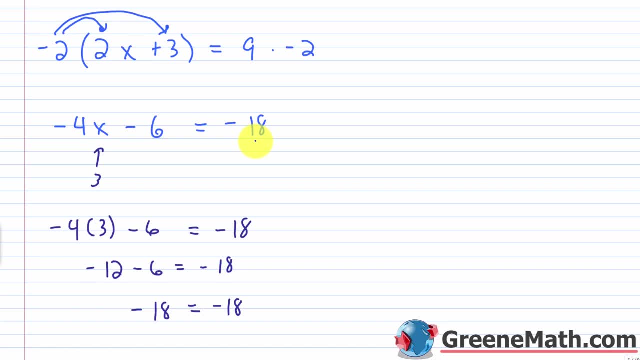 both sides of the equation by negative 2, the solution was still: X equals 3.. So multiplying both sides of the equation by the same non-zero value allowed us to keep the same solution Alright. so now that we've covered some of the basics, let's talk about the procedure to actually solve. 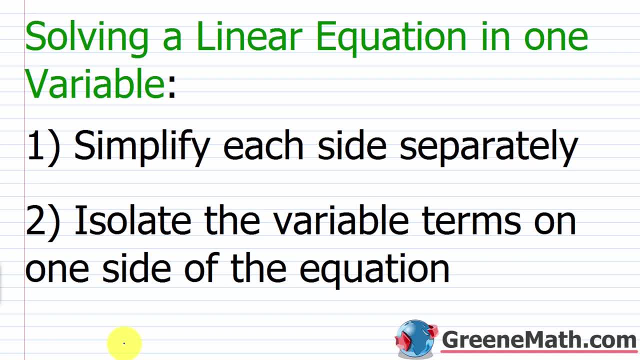 a linear equation of one variable. Before I start here, I just want you to put this down on a piece of paper. Your main goal is to isolate the variable. So you want X or Y or Z or whatever. the variable is on one side of the equation and you want a number on the other. 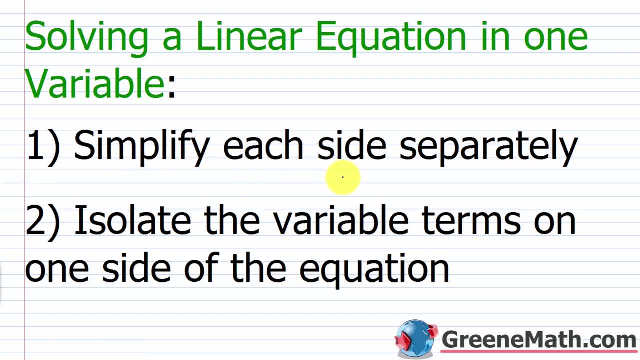 So this is how we go about doing that. We want to simplify each side separately. So that means you're going to clear parentheses, combine like terms on each side. You just want to completely simplify each side. Then we want to isolate the variable terms on one side of the equation. 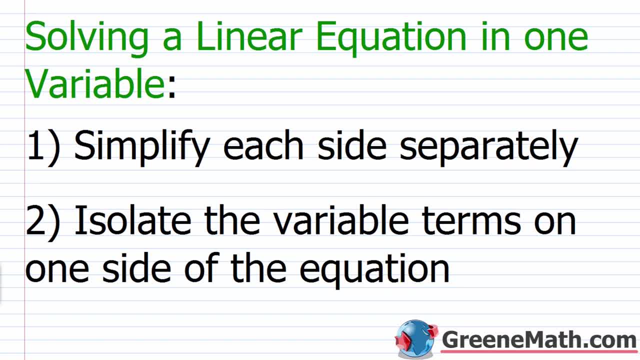 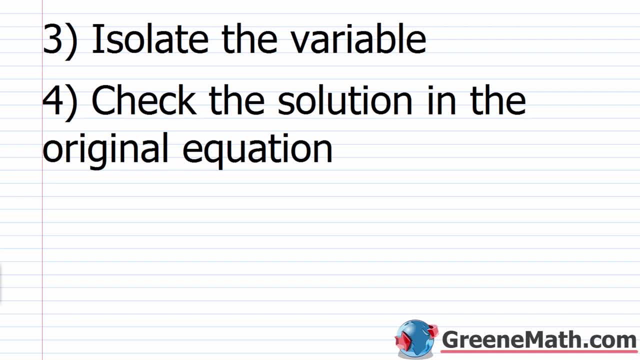 We're going to do this by using our addition property of equality. Then we want to isolate the variable, And we're going to do this using our multiplication property of equality, And then, lastly, we're going to check the solution in the original equation. So we take our solution. 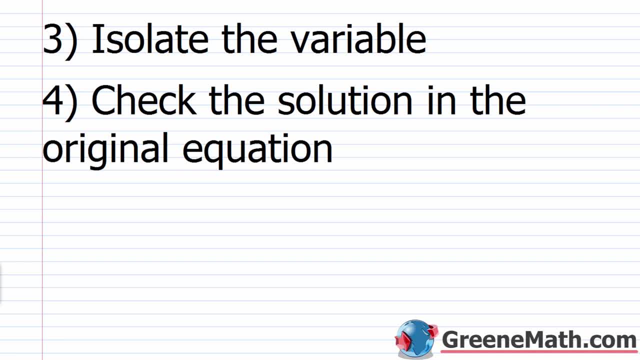 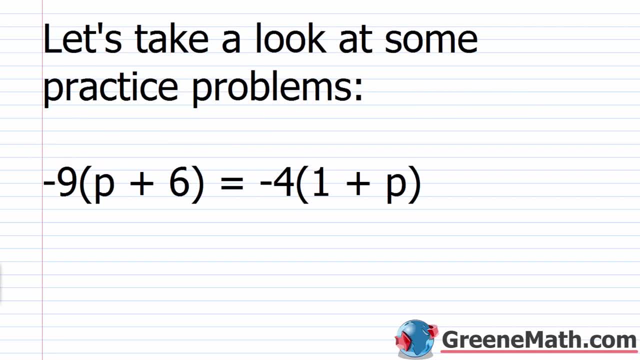 and we plug it back in for the variable in the original equation And we make sure that the left and the right side are equal. Alright, so let's go ahead and take a look at some practice problems, And we're going to start out with: we have negative nine times the quantity. 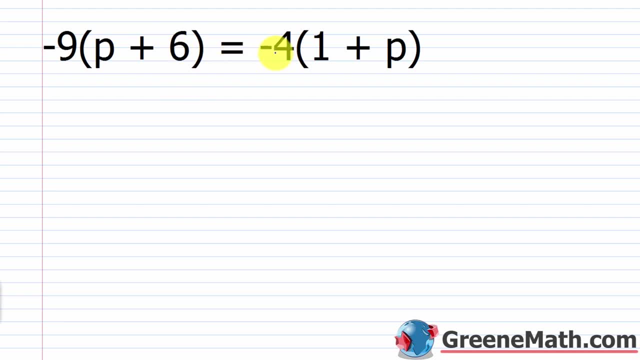 P plus six, This is equal to negative four times the quantity one plus P. So our variable here- and I'll just highlight it- is P. So what we want to do is start out by simplifying each side separately. So I'm going to use 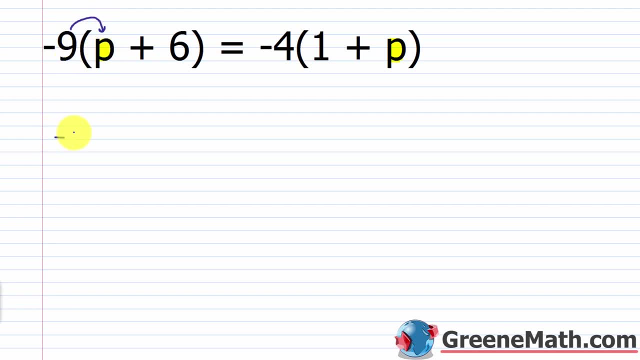 my distributive property here. Negative nine times P is negative nine P. Then I have negative nine times six and that's negative fifty-four. So then this is equal to- I'm going to use my distributive property over here. Negative four times one is. 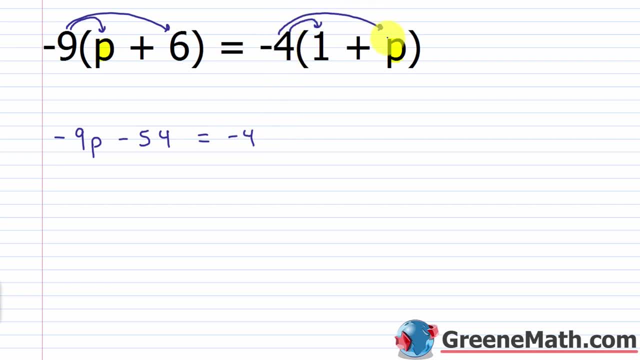 negative four And then negative four times P is minus four P. So now that I've got it in this format- remember- I want to isolate the variable terms on one side of the equation. So a variable term just means a term with a variable involved. 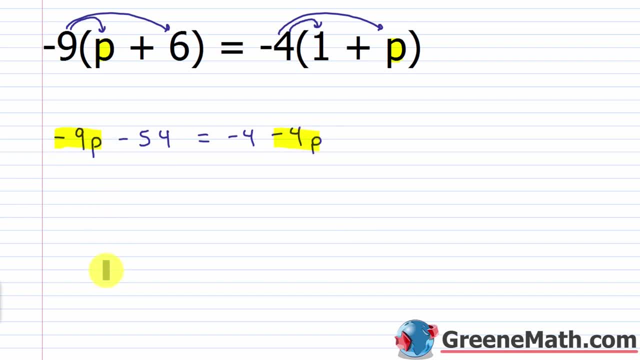 So that would be this term and this term. So what I can do is I can either move this over here or I can move this over there. Doesn't matter. What I'm going to do is I'm going to add four P to both sides of the equation. 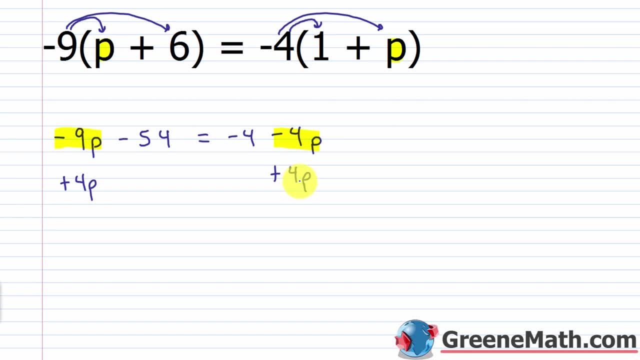 And what is that going to do? If I have negative four P plus positive four P, those two are going to cancel, right? This becomes zero. Now, over here, I would have negative nine P plus four P. That's negative five P, Then minus fifty-four. 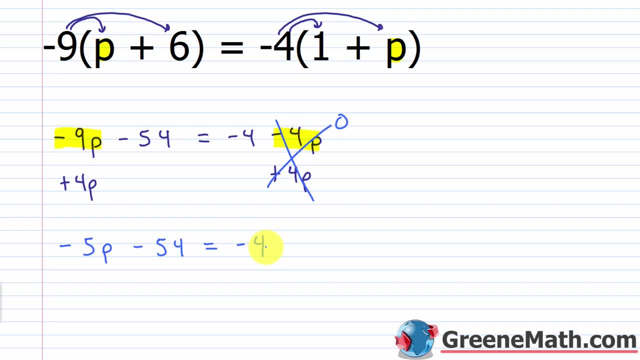 equals negative four. Now I want to isolate this term on this side of the equation And to do that. if I have this minus fifty-four here, I've got to get rid of it, And what I do is I want to use my addition. property of equality. 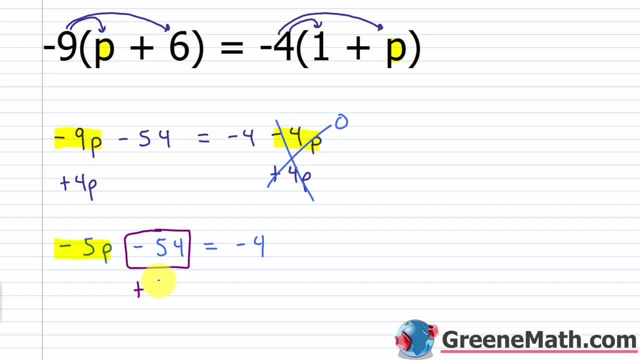 again. If I have minus fifty-four, I just add fifty-four to both sides of the equation. Negative fifty-four plus fifty-four is zero. That gets rid of that, And so what I'm left with here is negative five P by itself. 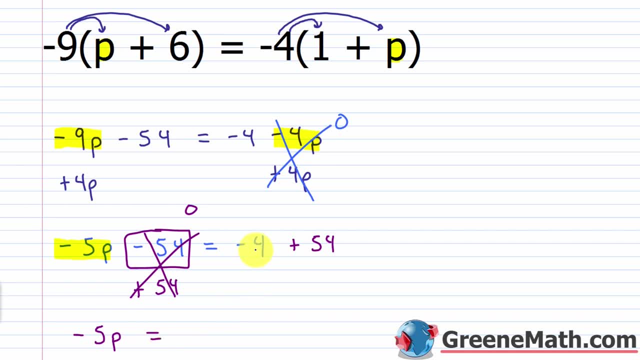 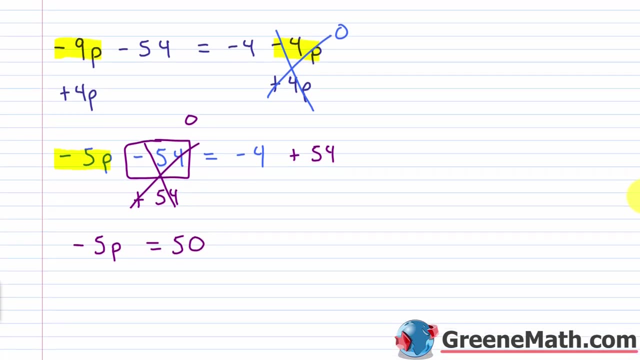 it's isolated on the left side is equal to negative four plus fifty-four Negative four plus fifty-four is fifty. Now the third step says we want to isolate the variable. How are we going to do that? Let's take a look at this variable, And I know a lot of you just know the answer to this because you solved a lot of these. 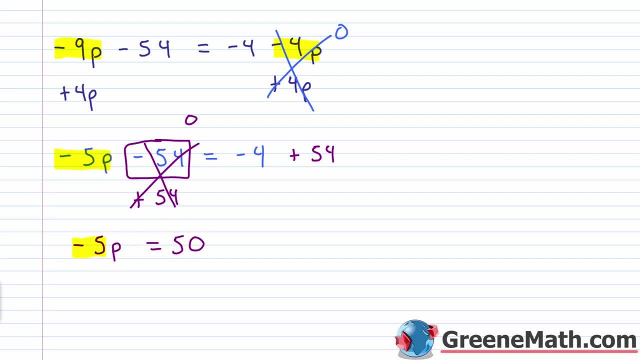 already. If I want to isolate that variable which is P, I've got to get rid of that negative five, That's the coefficient of P. Well, what's the opposite of multiplication If negative five is multiplying P, the opposite is division. So what I can do is 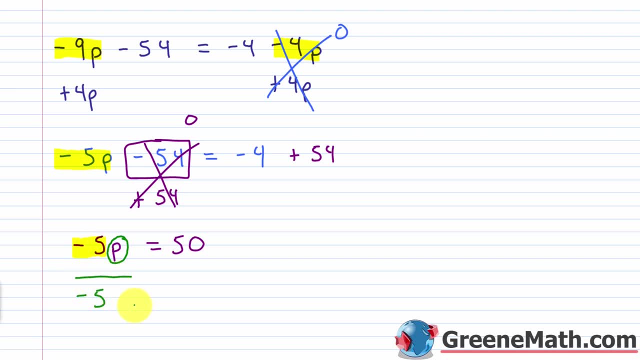 I can divide by negative five And what that does is any non-zero number divided by itself is one. So negative five over negative five is one. One times P is the same thing as P. Now, I can do this, provided I do it to the other side. 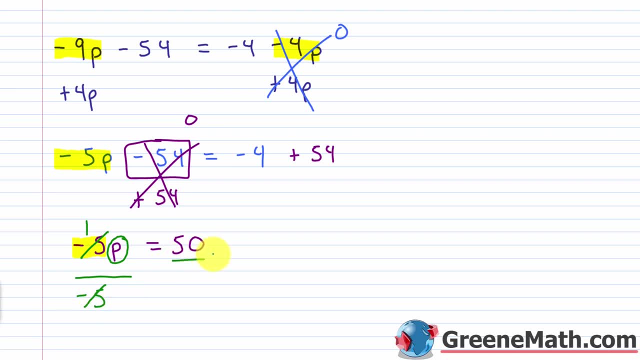 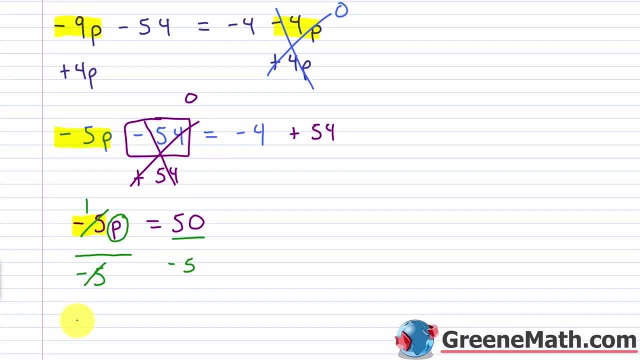 That's part of the multiplication property of equality. It extends to division, So I divide this side by negative five as well, to make it legal, And what I have is just P on the left side, On the right side, fifty divided by. 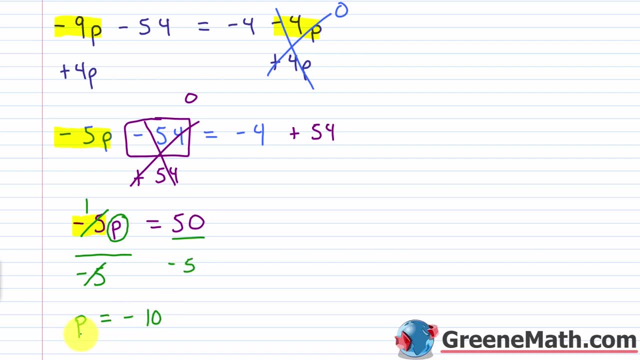 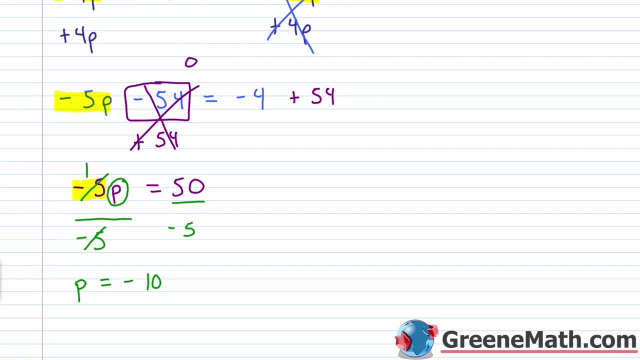 negative five is negative ten. So this is my solution: P equals negative ten, And at this point we're going to start writing things in solution set notation. And a solution set is just a set whose elements are solutions to our equation. So in this case, the set would have: 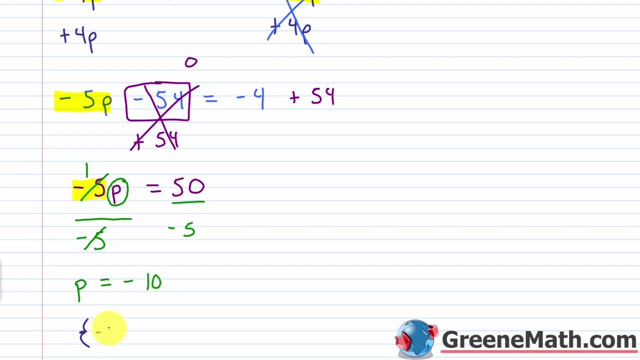 one element, And that element would be negative ten. So I just put negative ten inside of set braces, And so your teacher is still going to accept this as an answer. But more traditionally, as we move up we would write it using the set notation, So negative. 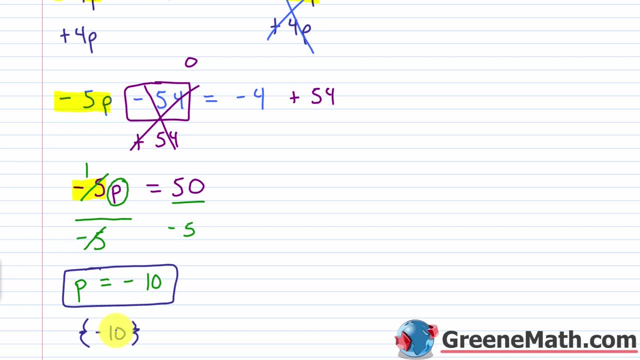 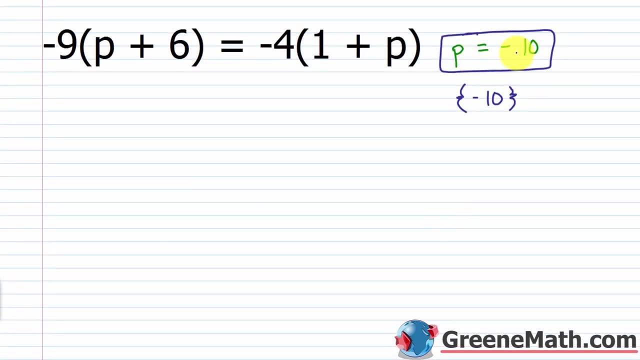 ten is our answer here. Now, what I want to do is I want to show you how to check this. Let me erase everything, Okay. so what I want to do is I want to plug in a negative ten. everywhere I see a P, So I'm going to plug a negative ten in here and also. 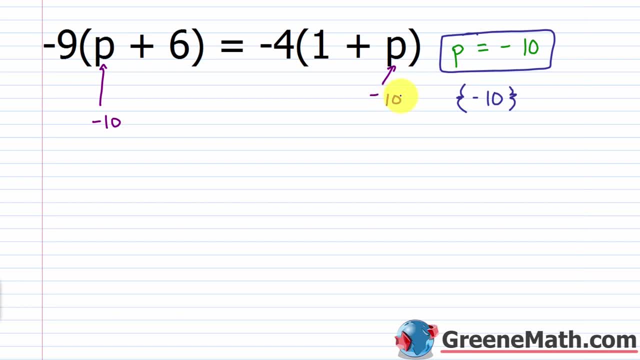 here And we want to make sure the left and the right side are equal to each other. So you'd have negative nine times the quantity negative ten plus six, And this is equal to negative four times the quantity one plus negative ten. Okay, So negative ten plus six is negative four. So you'd 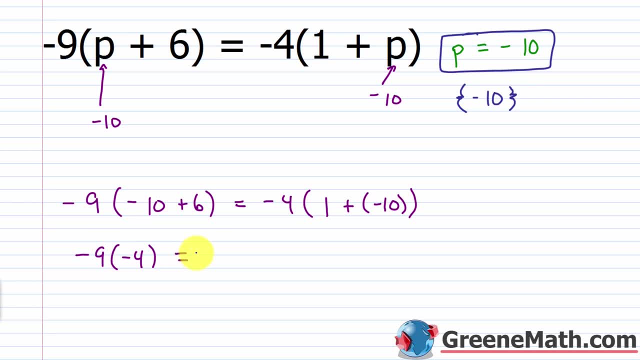 have negative nine times negative four, And this should be equal to, inside of here, one plus negative ten is negative nine. So you'd have negative four times negative nine. You can already see this is the same value. Negative nine times negative four is thirty-six. 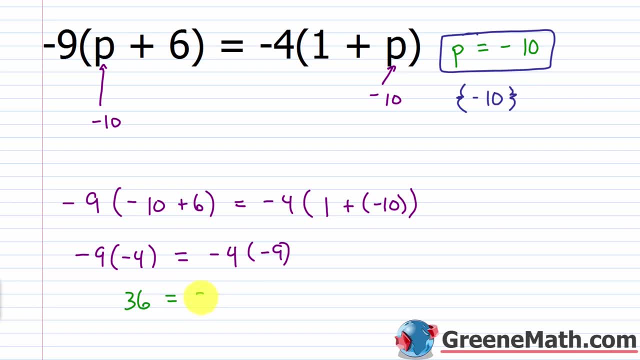 So you'd have: thirty-six on the left is equal to thirty-six on the right, So you have the same value on each side of the equation. So that tells you that your solution, which is P equals negative ten, is correct. Alright, let's take a look at the next example. So we have four R. 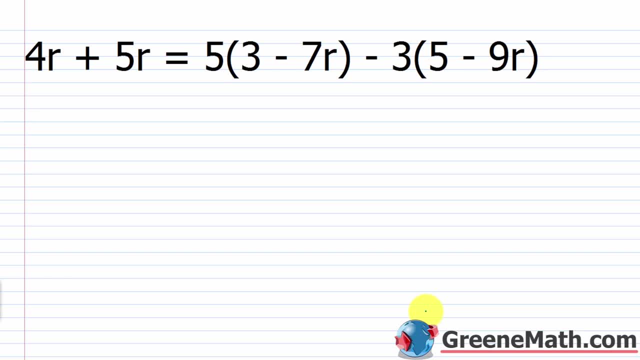 plus five R is equal to five times the quantity three minus seven R minus three times the quantity five R. So again I want to simplify each side separately. So four R plus five R is nine R. I'm just combining like terms there. This is nine R. 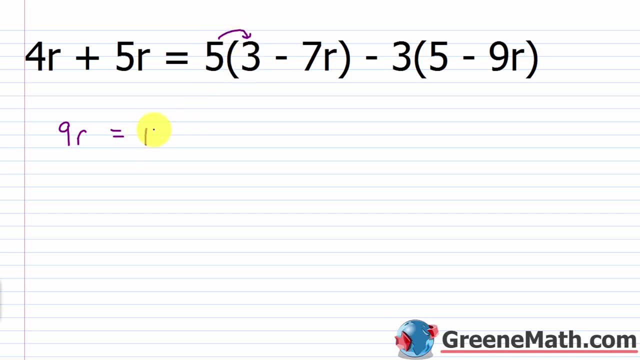 This is equal to using my distributive property here. five times three is fifteen minus five times seven, R is thirty-five R. And then I have- I might as well treat this as- negative three. So negative three times five is minus fifteen. And then negative three times negative nine R is: 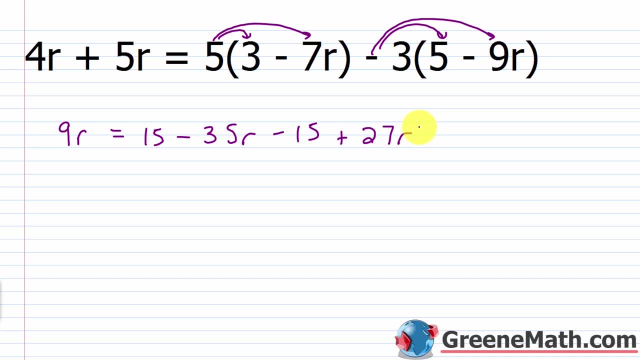 positive twenty-seven R, And then I can combine more like terms here: Fifteen minus fifteen is zero, So this would cancel. And then negative thirty-five R plus twenty-seven R is negative eight R. So you get that nine R is equal to negative eight. 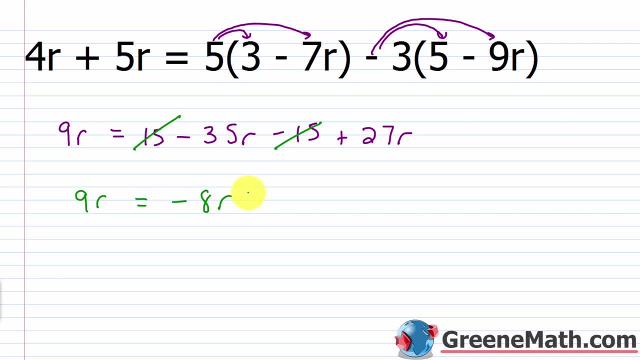 R. So now I want to move all my variable terms to one side. So in this equation I just have variable terms, I have nine R and I have negative eight R. So what I'm going to do is I'm just going to add. 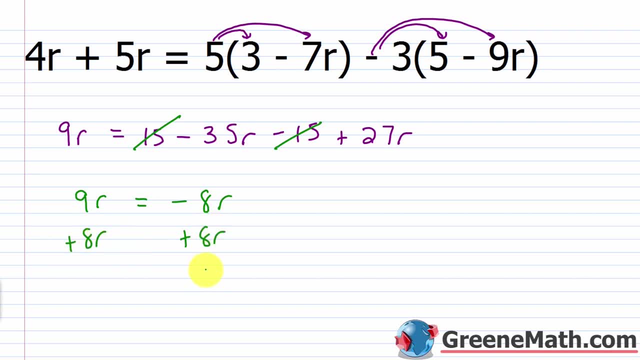 eight R to this side of the equation. If I have negative eight R plus eight R, this becomes zero. Make sure you write zero. That's very important. So put zero here And then over here I'll have nine R plus eight R, which is seventeen R. 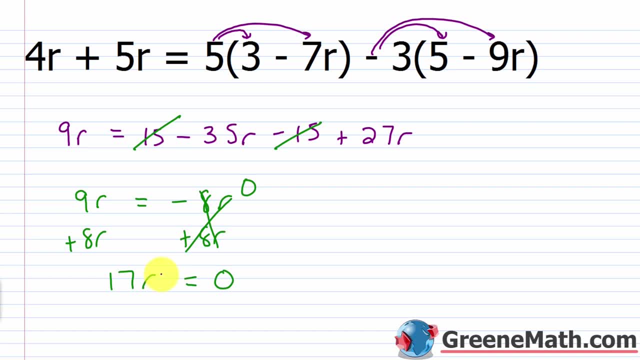 Now I want to isolate the variable. In order to do that again, if I want to isolate R and seventeen is multiplying R to get R by itself, I divide both sides of the equation by seventeen. This will cancel with this and become one, So I'll have one. 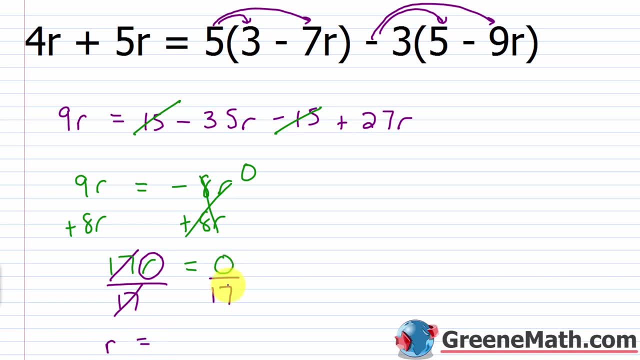 R or just R, And this will be equal to zero over seventeen, which is zero. So my solution set contains one element, and that element is zero. Now, if you want to check this- I'm not going to in the interest of time- All you want to do is plug a zero in for each R. 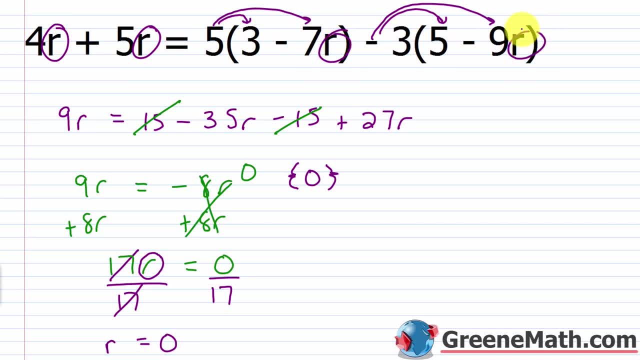 in the original equation. So there, there, there and there, And you'll see that the left and the right side will give you the same value, And that's how you know your solution is correct. Alright, let's take a look at another one. 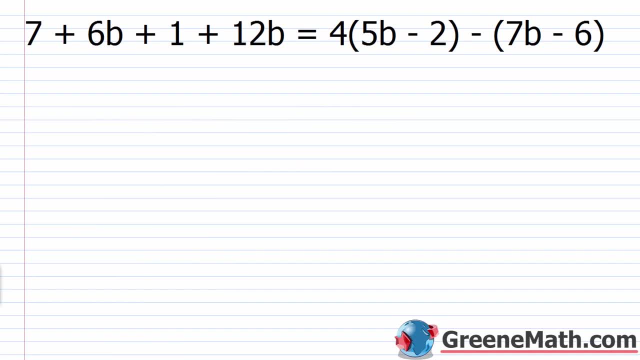 So we have seven plus six B plus one plus twelve B is equal to four times the quantity five B minus two minus the quantity seven B minus six. So on this side I can combine these two and these two. Seven plus one is eight. Six B plus twelve B is eighteen B. 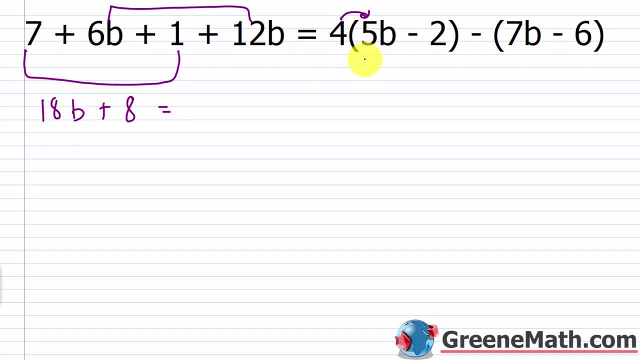 Over here I use my distributive property. Four times five B is twenty B. Then minus four times two is eight. Then I'm going to treat this as a phantom negative one. So instead of having this minus out here, I'm going to put 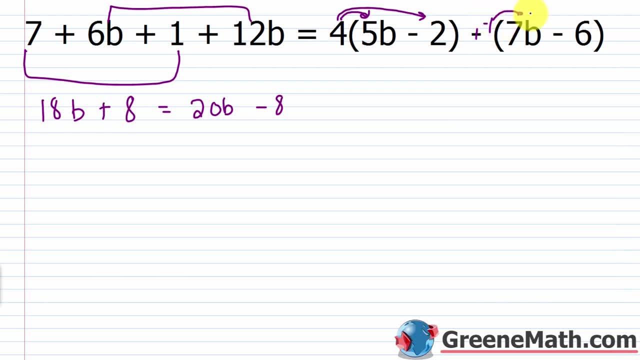 plus negative one, And I'm going to use my distributive property: Negative one times seven B is minus seven B, And then negative one times negative six is plus six. So over here I can think about: twenty B minus seven B is thirteen B. Okay, this is. 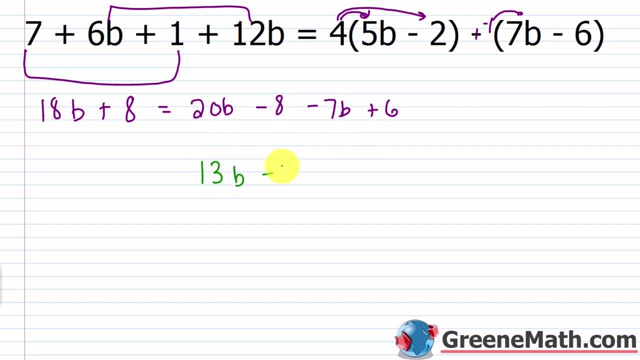 thirteen B And then negative. eight plus six is negative two. So now again I want to bring all the variable terms to one side and I want all the numbers on the other. So I'm going to subtract thirteen B away from each side of the equation. 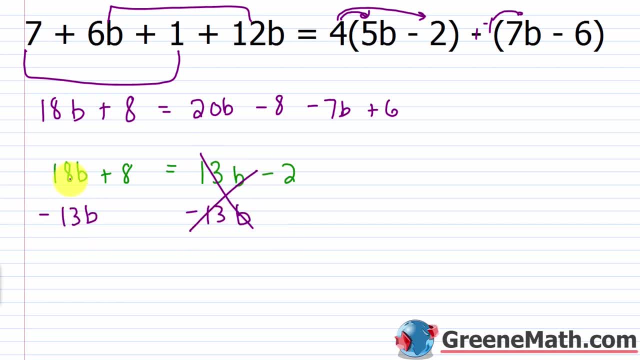 so that this is gone. So eighteen B minus thirteen B is five B, And I'm also going to subtract eight away from each side of the equation, So this is gone. So I'll put equals negative. two minus eight is negative ten, So now I have a variable term. 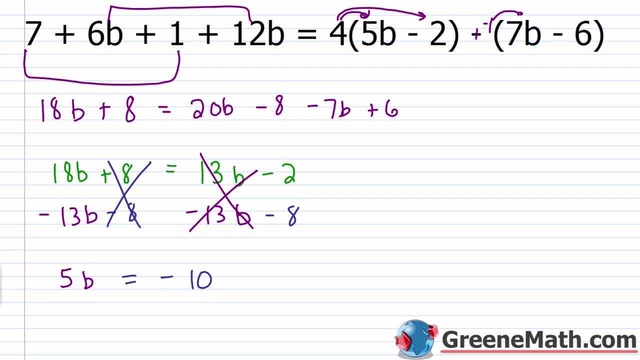 on one side and a number on the other. All I need to do at this point is isolate the variable. So I want to isolate B. And again, if I want to isolate B and five is multiplying B? I just divide by five. Okay, I divide by five. 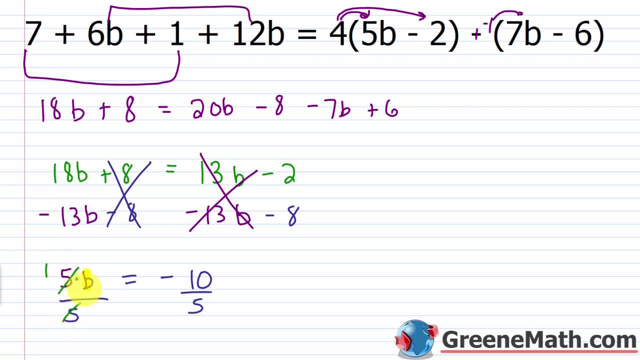 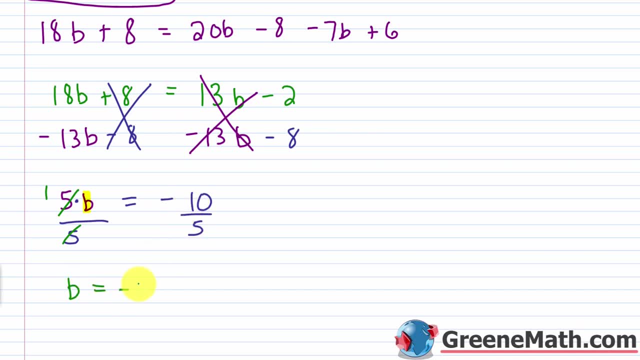 This is going to cancel with this and become a one. One times B is the same as B, So I've isolated the variable. So I'll have: B is equal to negative ten over five, which is negative two. So my solution set here will contain one element. 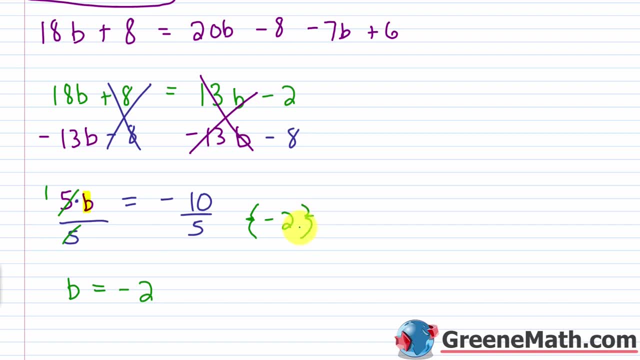 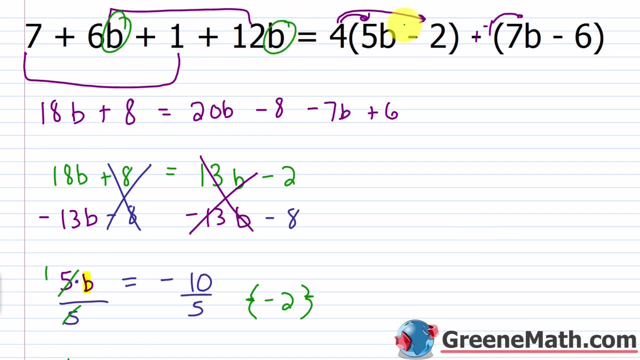 just negative two. Now again, if you want to check this in the original equation, go everywhere. you see a, B. So here, here, here and here, Plug in a negative two and you'll see that the left and the right side are equal, and so we'll know that our solution: here: B equals negative two. 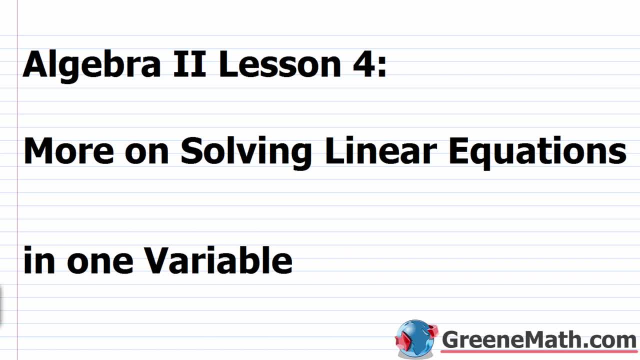 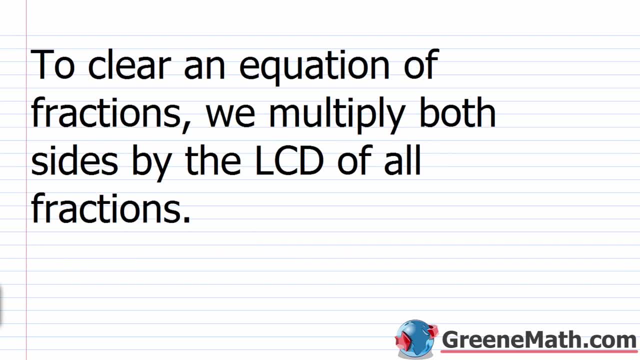 is correct. Hello and welcome to Algebra 2, Lesson 4.. In this video, we're going to continue learning about solving linear equations in one variable. So now we're going to deal with some special case scenarios. So the first thing I want to talk about today 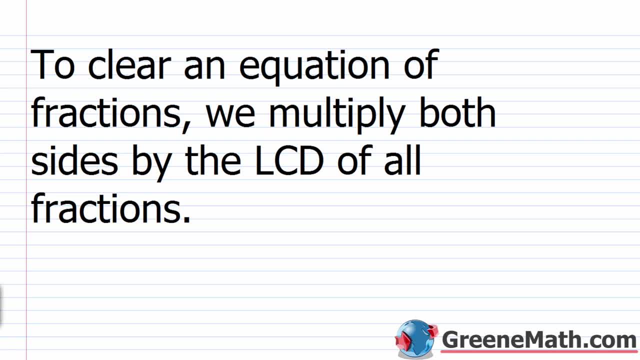 is what to do when you have a linear equation in one variable and you have fractions involved. So typically, to make it easier on ourselves, we want to clear the equation of fractions before we begin, But, as I'm going to show you with this first example, you don't have to do that. Okay, you'll get the same answer. 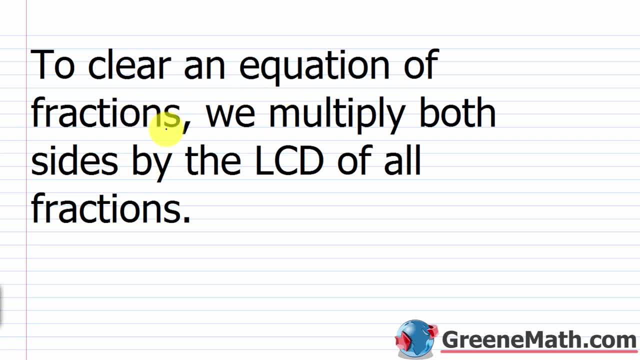 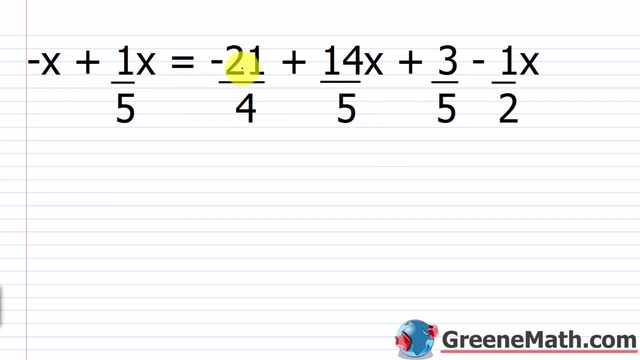 either way. So to clear an equation of fractions, we multiply both sides by the LCD. that's the least common denominator of all fractions. So here is an example. I have negative x plus one-fifth x is equal to negative twenty-one. 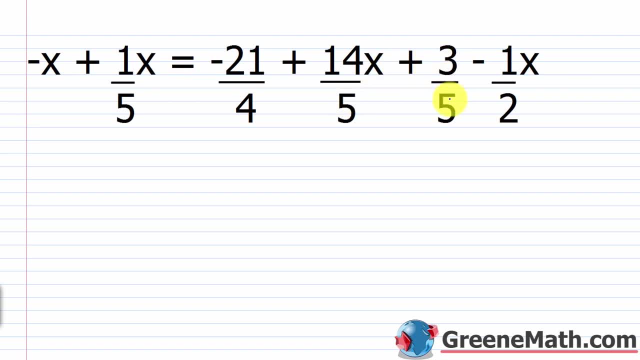 fourths plus fourteen-fifths x plus three-fifths minus one-half x. So to not deal with these fractions, I can just figure out what the LCD is. So I have a five, I have a four, another five, another five and a. 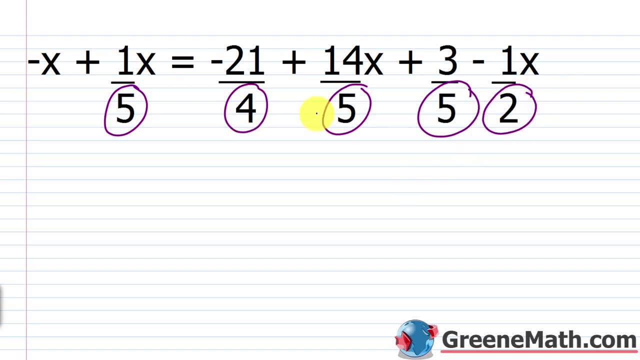 two. Now, really, the only thing I need to think about is the five and the four. Five times four is twenty, so the LCD here would be twenty. So what I want to do is I want to multiply both sides of the equation by this number twenty. 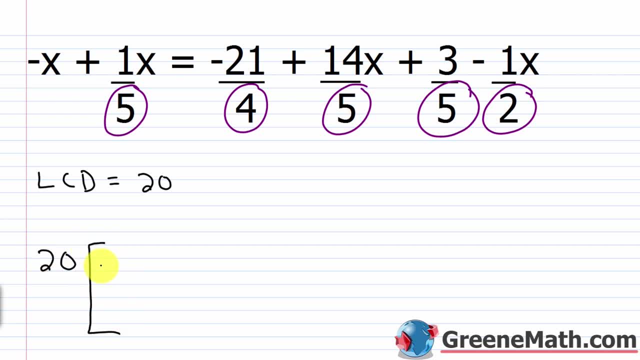 So let me just copy everything. So it's negative x plus one-fifth x, and then I'll close the brackets there and then I'll put equals, put some new brackets. we'll have negative twenty-one fourths and then plus fourteen. 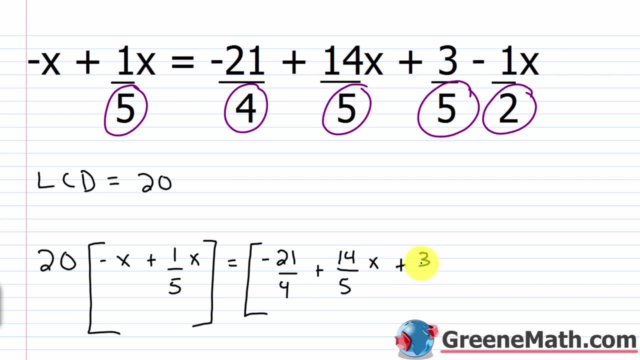 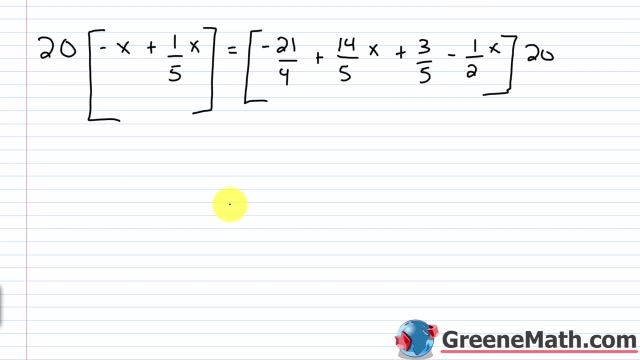 fifths x, then plus three fifths and then minus one-half x, close the brackets and then we're multiplying this by twenty. Alright, let's scroll down and get a little room going, So I'm going to use my distributive property. I'd have twenty. 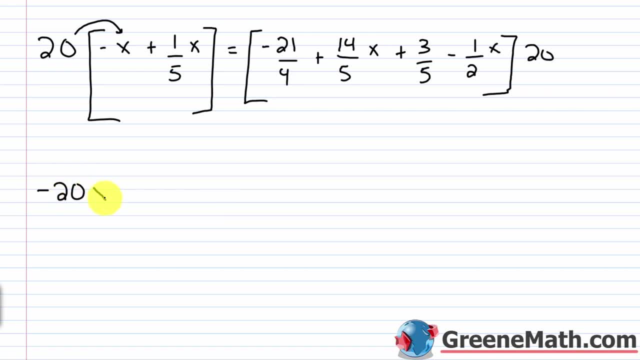 times negative x. That would be negative twenty x. And then next I'd have twenty times one-fifth x. So let me write that out: So plus twenty times one-fifth x. So here's where we're going to do some canceling This. 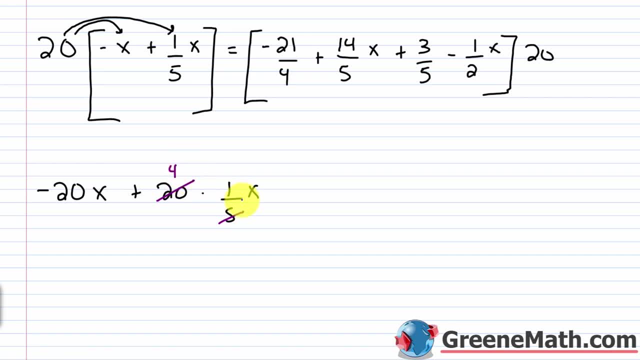 twenty would cancel with this five and give me a four. Then four times one x or four times just x is four x. So let me erase this and just put four x. Okay, then we have equals. Now next I have twenty. that's going. 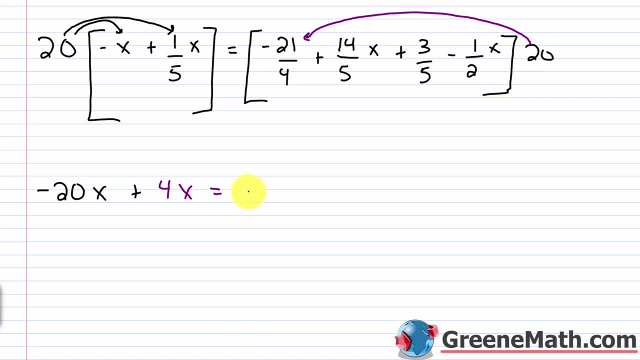 to multiply negative twenty-one fourths. So let's write that out: So negative twenty-one fourths times twenty, And of course I can do some canceling here. This twenty will cancel with this four and give me a five. Five times negative. twenty-one is negative one-hundred. 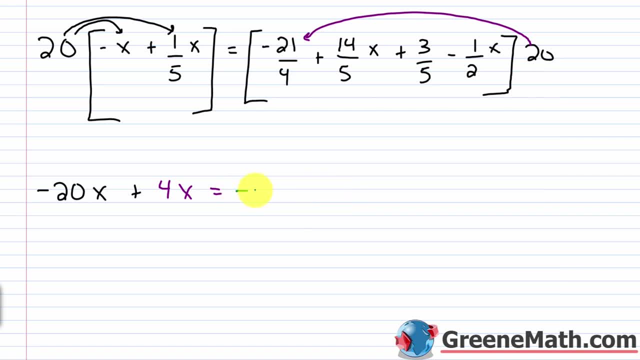 five. Let's erase this and put negative one-hundred five. Then I'll have twenty times fourteen-fifths x. So plus twenty times fourteen-fifths x, And what's going to happen is this twenty will cancel with this five and give me a four Four times fourteen. 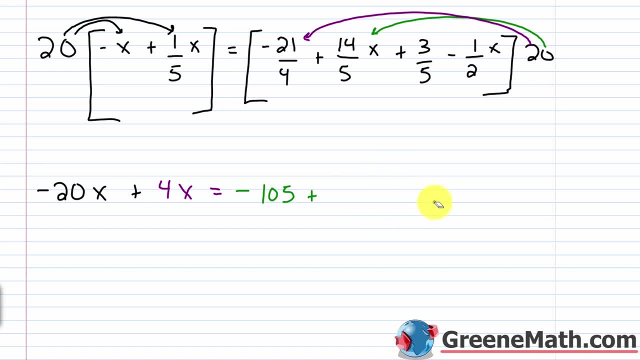 is fifty-six, Then times x is just fifty-six x. Let's write fifty-six x here, And then I have twenty times three-fifths. So plus twenty times three-fifths, And this will cancel with this and give me a four. 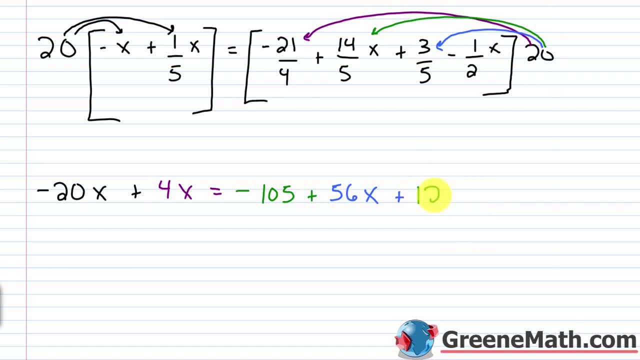 Four times three is twelve, So this would be twelve. And then, lastly, I'll have twenty times negative, one-half x, So I'll put minus one-half x times twenty, And again this will cancel with this and give me a ten, Ten times negative. one is: 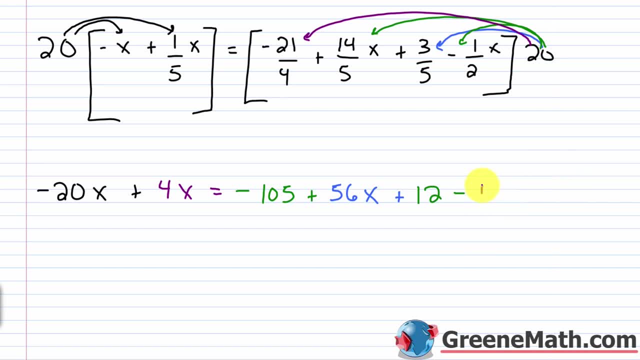 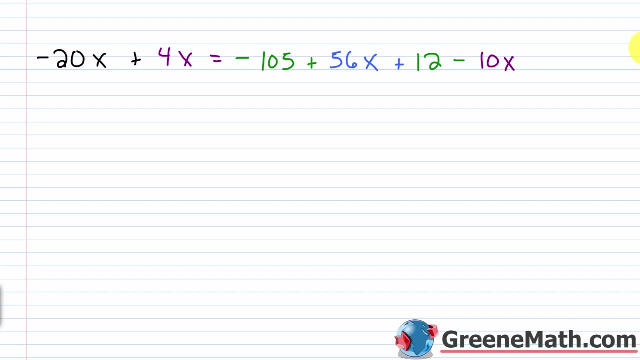 negative ten. So this would be minus ten x. So minus ten x. So it took a while, but we've cleared our equation of fractions And now what we can do is just proceed as we normally do. We would simplify the two sides separately. On the left side I have negative. 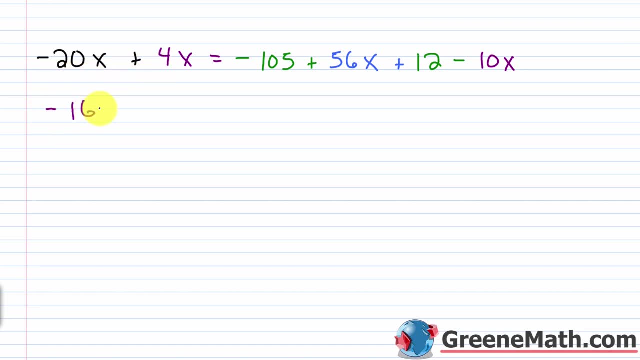 twenty x plus four x, That is negative sixteen x. On the right side I can combine fifty-six x and negative ten x. That would give me forty-six x. Then over here, negative one-hundred five plus twelve is negative ninety-three. So this would be forty-six x. 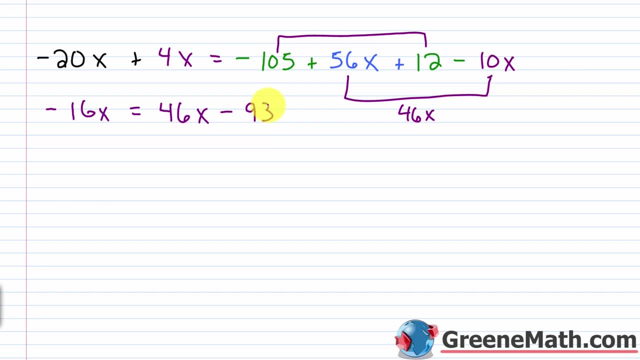 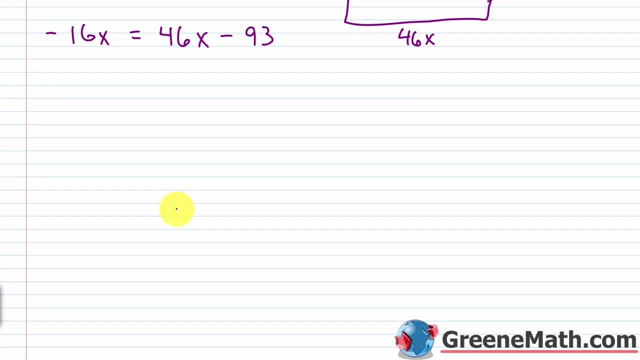 Minus ninety-three, And let me scroll down and get a little room going. So now what I want to do is put all the variable terms on one side and the numbers on the other. Really, all I need to do is subtract forty-six x away from each side of the equation. 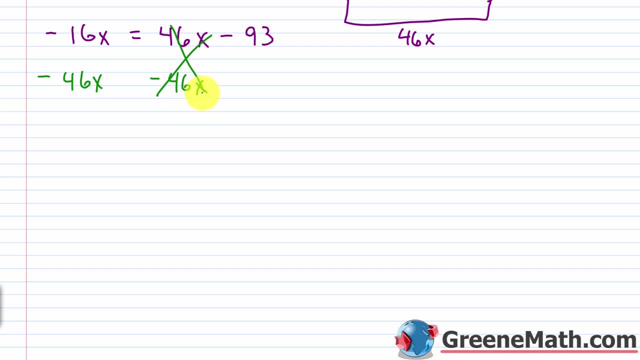 So this is going to cancel Negative sixteen x minus forty-six x is negative sixty-two x And this equals negative ninety-three. One last step for us here: We want to divide both sides of the equation by negative sixty-two, So we can isolate our variable. 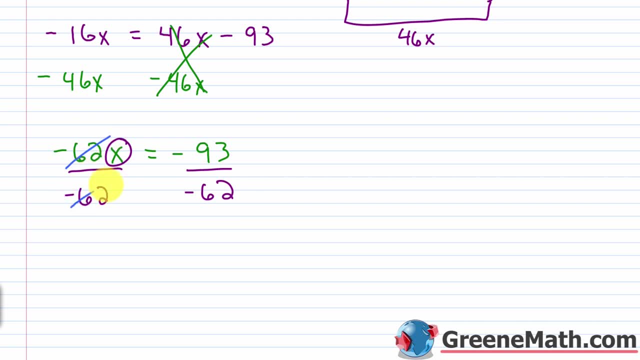 x. So what's going to happen is this: will cancel with this and give me a one. So I have x by itself And this equals we have negative ninety-three over negative sixty-two. Let's see if we can reduce that any. I know that negative ninety-three. I could write this as: 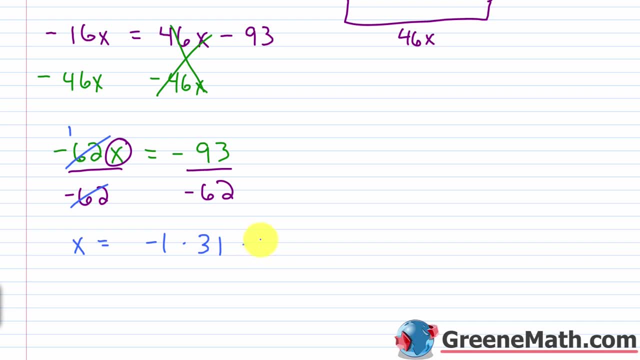 negative one times thirty-one times three And I know that negative sixty-two. I could write this as negative one times thirty-one times two, So we can see that we can cancel the negative one with the negative one. Obviously, negative over negative is positive. 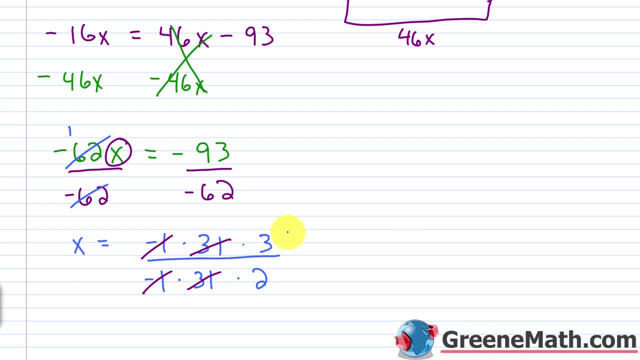 We can cancel the common factor of thirty-one And what I'm left with here is three halves. So I can erase this and just put: x is equal to three halves. So again we've been using this solution, set notation, and so inside of set braces, I would just list: 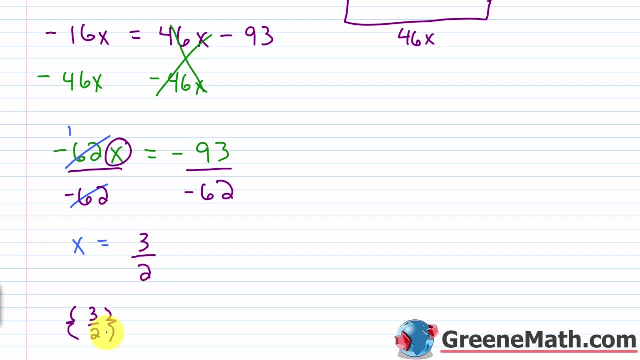 three halves and we're done there. Now, normally in algebra one- I checked everything- I would go back and I would substitute three halves in for x and it would show you the left and the right side are equal. As these problems get more complex, it's more time consuming to do that. So my strategy: 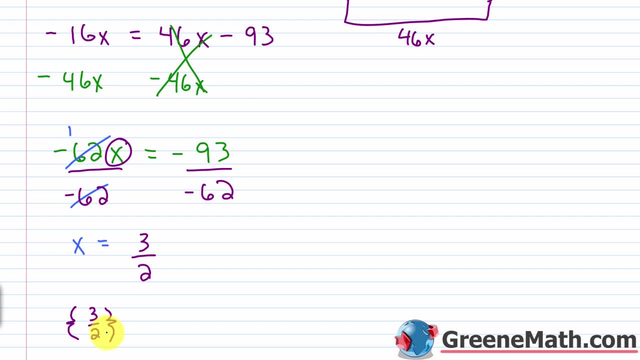 for you is: pause the video. go ahead and check it Now. if you're on a timed examination, you might say: hey, what do I do? Should I check everything and not finish the whole test? The answer to that is no, If you have. 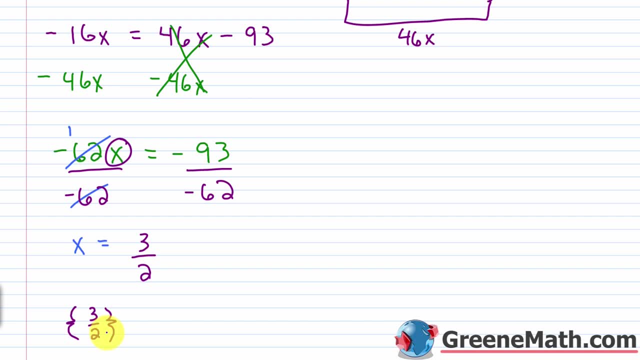 a lot to do on your test. complete the test. Don't check anything Once you're done, where students would normally rush up to hand in their paper and run out of the classroom. take the extra time to go back and check the ones that you're unsure of. You do those first. 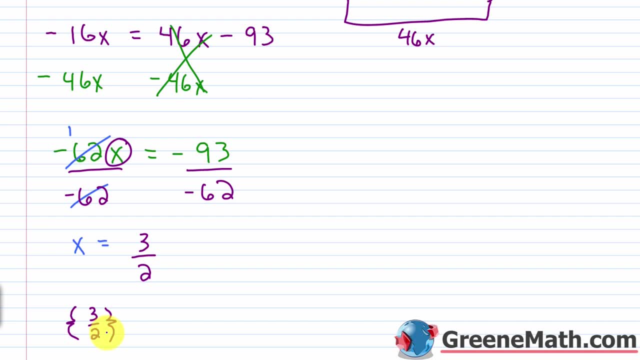 Then you go back and you check as many other problems as you can. Hopefully you can check all of them and you'll catch any silly mistakes that you've made. Now I want to show you one thing before we kind of move on to the next example. Let me erase everything, So I want to quickly. 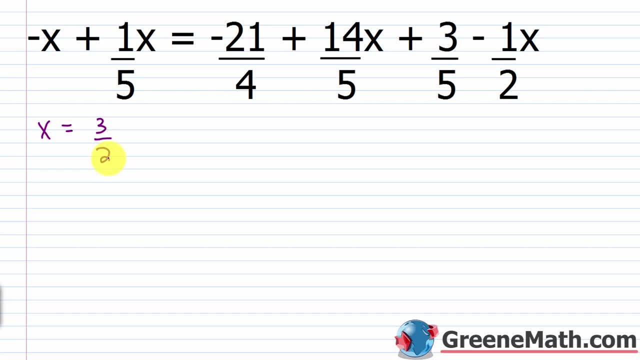 show you that you get the same answer whether you clear the equation of fractions or you don't. So over here I have negative x plus one fifth x. To get a common denominator going, I could just multiply this by five over five, and what would that give me? It would give me negative five x plus. 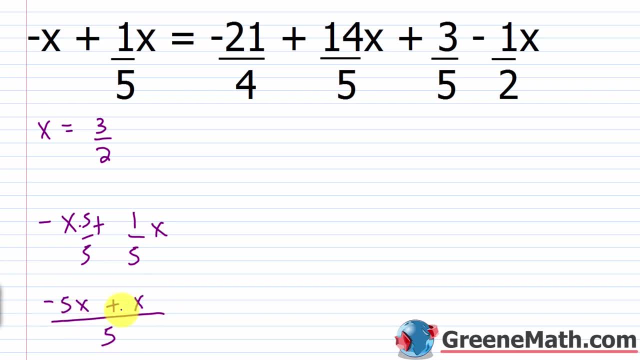 x over five. Well, this would be negative. four x right Negative. five x plus x is negative. four x over the common denominator of five. So that's the left side. So negative four x, negative. four x over five. Now this is equal to over here. 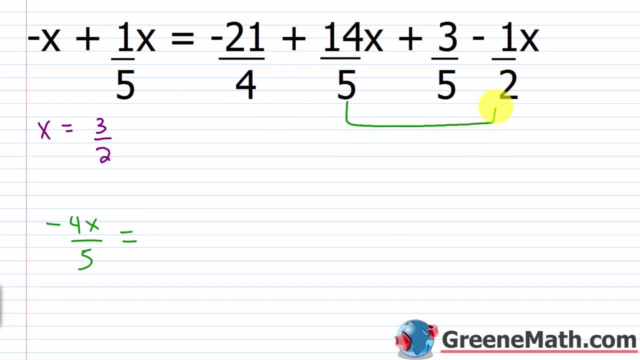 to get a common denominator between here and here. I see I have a five and a two. So if I multiply this by two over two and I multiply this by five over two, five over five, what I'm going to have is twenty-eight x over ten minus. 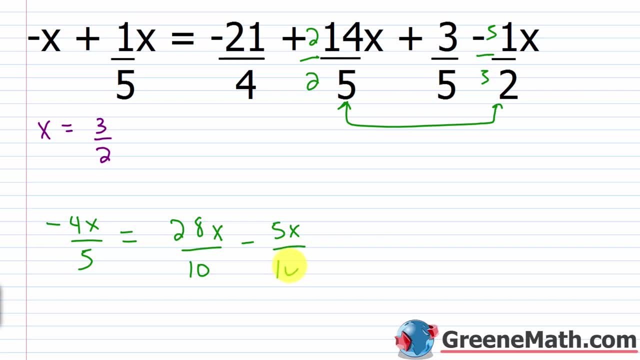 over here. I have five x over ten, So I have a common denominator. Twenty-eight minus five is twenty-three, So this would be twenty-three x over ten. So twenty-three x over ten. Let me erase that. And now the other thing we have to deal with is this: right here. 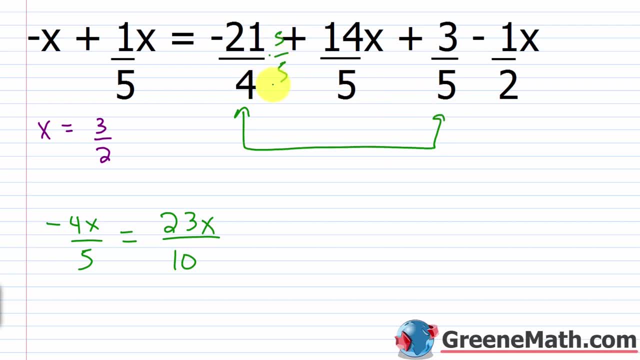 If I get a common denominator here, I multiply this by five over five and this by four over four, And what would happen is I'd have negative twenty-one times five, So that would be minus one hundred five over twenty, And then plus three times four is twelve, So twelve over twenty. 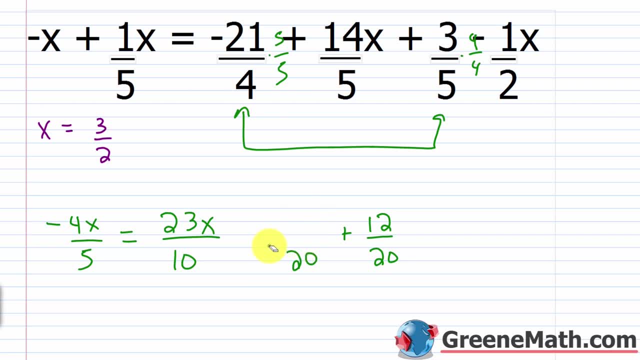 So if I sum negative one hundred five plus twelve, I get negative ninety-three. So this would be negative or minus ninety-three over twenty. Now let me scroll down and get a little room To get all the variable terms on one side. I would just simply: 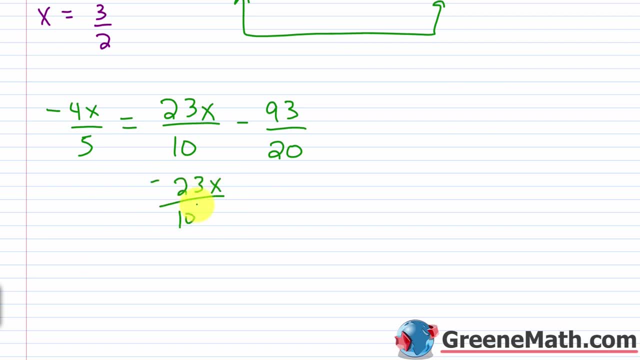 subtract twenty-three x over ten, away from each side of the equation, And of course to do that I need to have a common denominator. So I would take negative four fifths times x and I'd multiply this by two over two, And that would give me negative eight tenths. 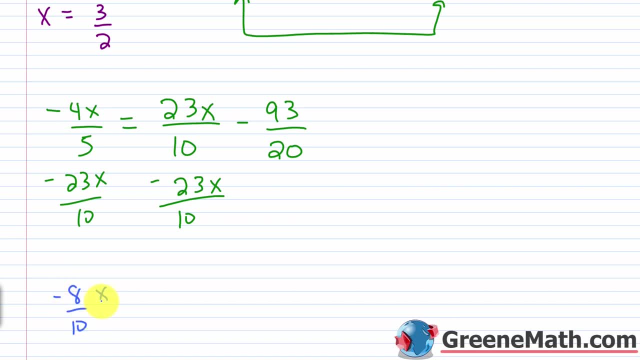 negative eight tenths x and then minus twenty-three x over ten. So when we look at this, really, we think about negative eight minus twenty-three and that's negative thirty-one. So what's going to happen here? this is going to become on the left side. 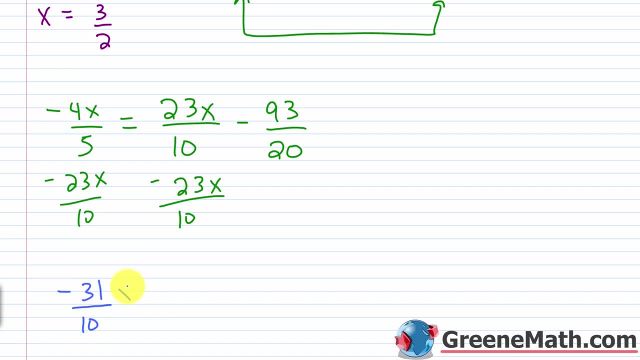 negative thirty-one over ten, and this is times x. This is going to cancel over here and be zero. So this will be equal to negative ninety-three over twenty. Now, how do I get my solution here? Let me scroll down a little bit. 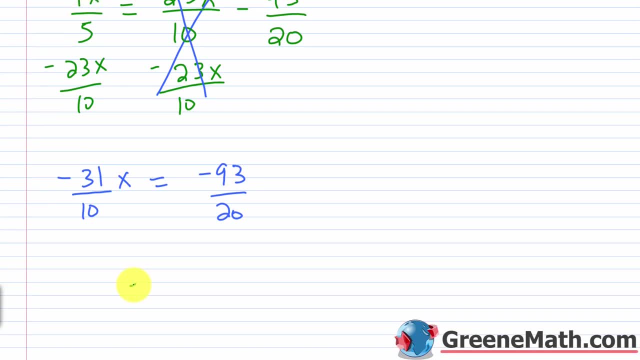 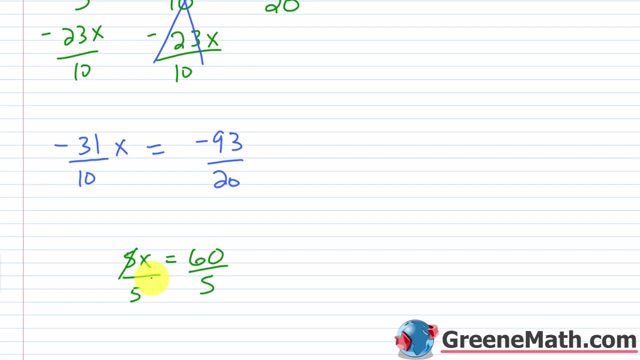 In most cases we see something like this. We see, you know, five x equals sixty, And we divide both sides of the equation by five, That's the coefficient of x. This cancels with this and I get: x is equal to twelve. But in this case we don't have something. 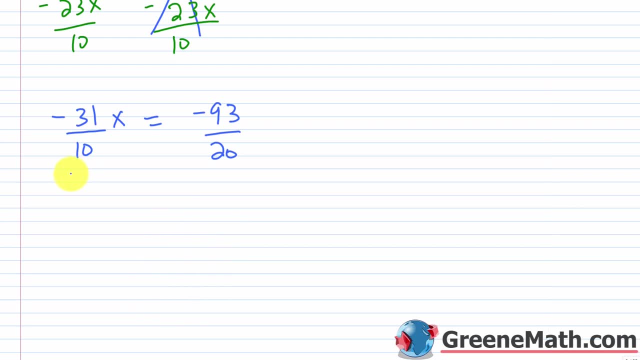 that looks like that, But we really do. I can still divide both sides of the equation by negative thirty-one over ten. But there's a quicker way to do that: You multiply by the reciprocal. So when your coefficient for x is a fraction, you multiply by. 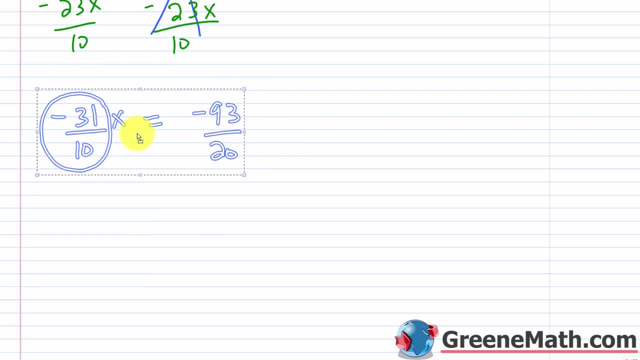 the reciprocal. Remember, all I'm trying to do is get x by itself, And multiplying something by its reciprocal makes it equal to one. So if I multiply this by negative ten over thirty-one, the negatives would cancel, and then ten would cancel with ten. 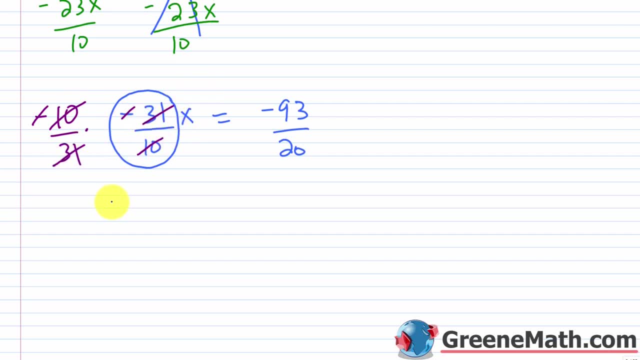 Thirty-one would cancel with thirty-one, So this is one times x, or just x is equal to. I've got to multiply by the same thing over here, so that's legal. So times negative ten over thirty-one. We know already that the negatives would cancel And we know that. 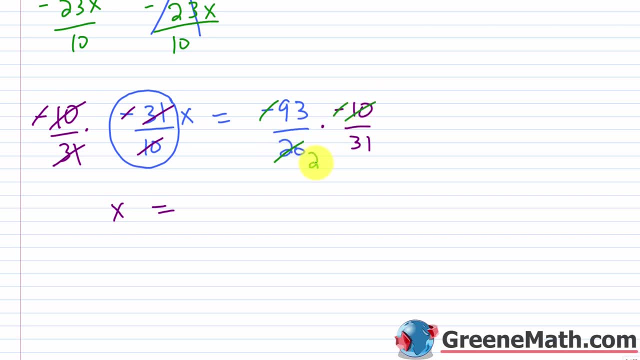 if I think about twenty and ten, this would cancel with this and leave me with a two Between ninety-three and thirty-one. this would cancel with this and give me a three. So I end up with x equals three halves, just like I did, okay, when we looked at it, by clearing the equation. 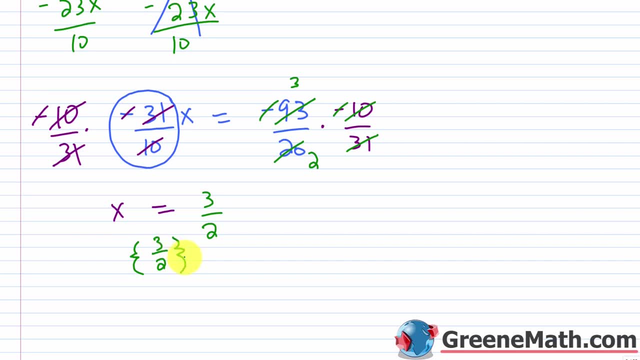 of fractions. Now, in this particular case, you could make the argument that it wasn't any faster to clear the equation of fractions. But I think, especially if you have kind of a simpler problem, it kind of is. So it's a personal preference whether you want to. 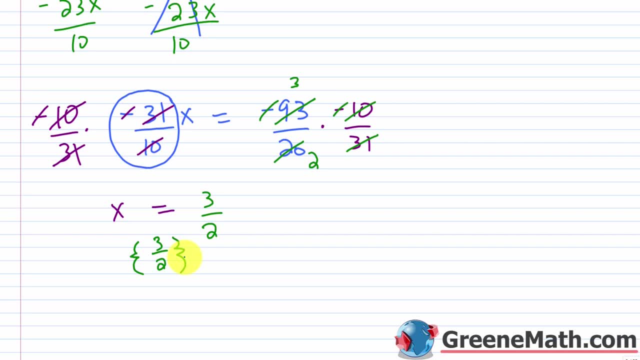 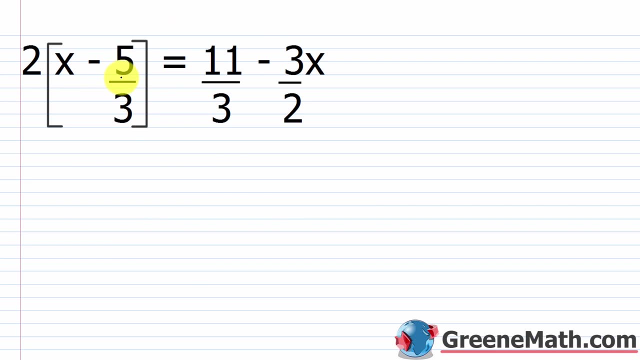 work with the fractions, or you don't want to work with the fractions, But in either scenario you're going to get the same answer. Alright, for the next one, I'm looking at two times. the quantity x minus five-thirds is equal to eleven-thirds minus three-halves x. Now 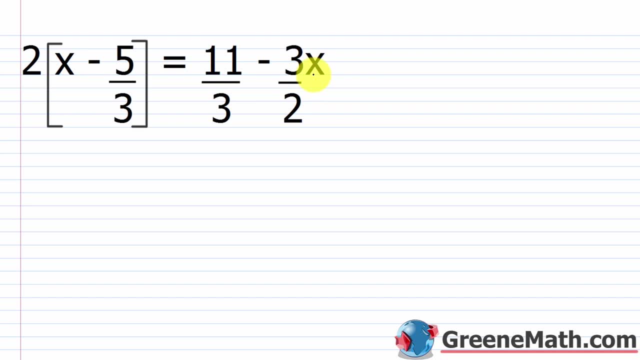 if you have a problem, okay, where there's fractions involved, you don't want to clear anything until you have removed all the parentheses and brackets, all the grouping symbols that you have to deal with. So what I would do here to start the problem. 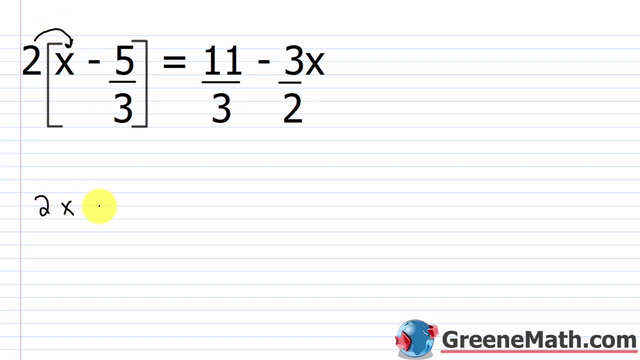 multiply two times x, that's two x. then minus, you'd have two times five-thirds. that would be minus ten-thirds. then this equals eleven-thirds and this is minus three-halves x. Now it's very easy to clear the fractions. now We come through here. 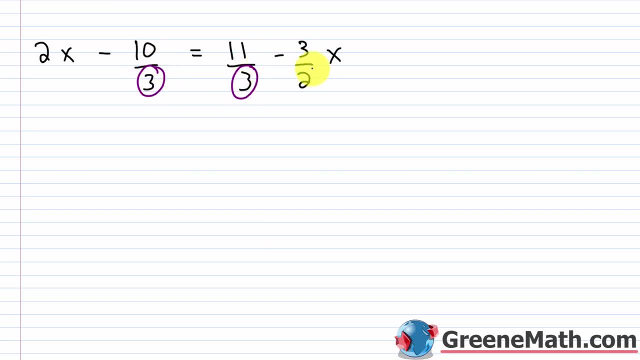 and we look at the denominators, I have a three, a three and a two. So what is my LCD? Well, it's just three times two, which is six. Now if I multiply both sides of the equation by six, I'm going to get what? So two x minus ten-thirds. 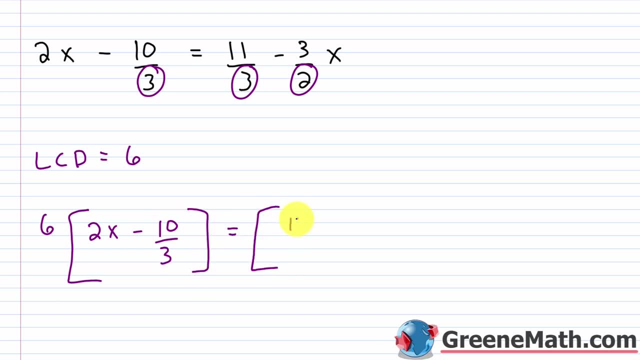 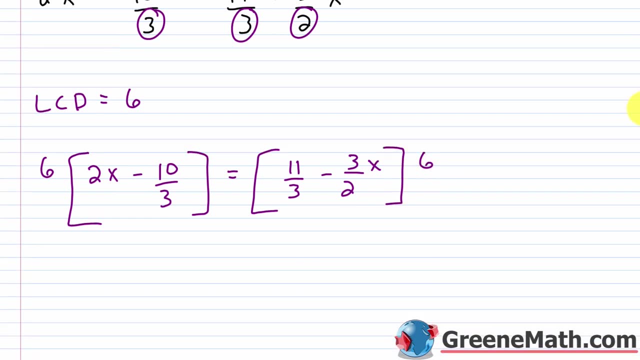 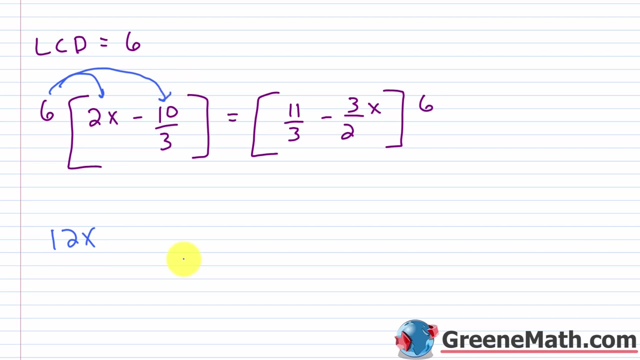 equals ten-thirds, That equals eleven-thirds minus three-halves x. Multiply this by six as well, So let's go ahead and crank this out. So six times two x is twelve x. Six times negative ten-thirds. So let's put minus six times. 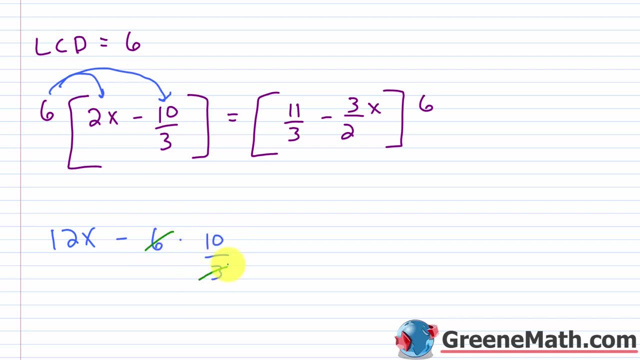 ten-thirds And we know that the six would cancel with the three and give me a two. Two times ten is twenty. This would be minus twenty here And this equals we have six times eleven-thirds. So six times eleven-thirds Six. 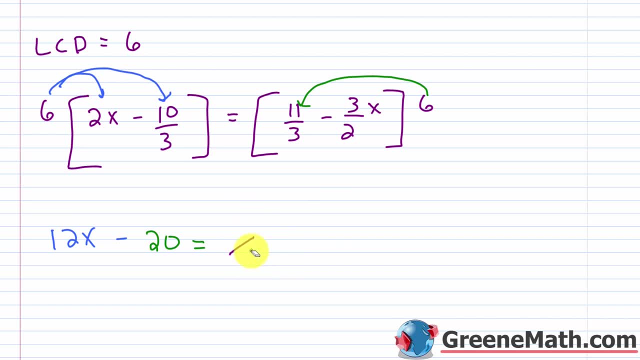 would cancel with three and give me a two. Two times eleven is twenty-two, So this is twenty-two. And then last we have six times negative three-halves x. So minus six times three-halves x, And this is going to cancel with. 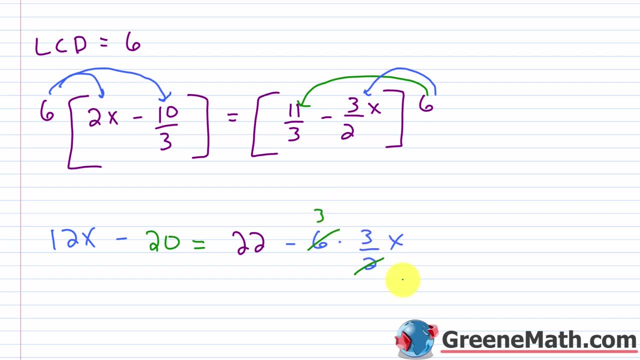 this and give me a three. Three times three is nine, So it would be minus nine x. Okay, So now we're done with that And we have an equation without any fractions involved. I want all my variable terms on one side, all my numbers on the other. 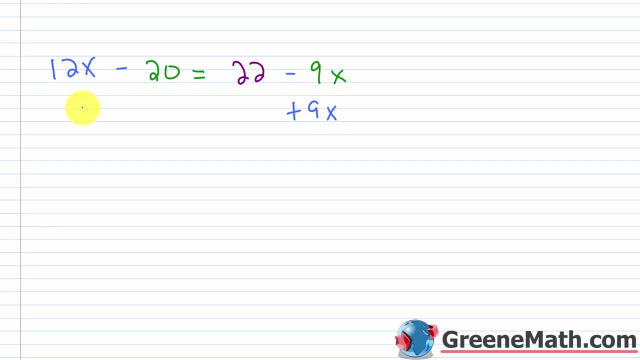 So let me add nine x to each side of the equation, So this is going to cancel and become zero. And then also let me add twenty to each side of the equation, So this will become zero, And twelve x plus nine x is twenty-one x, And this is equal to twenty-two. 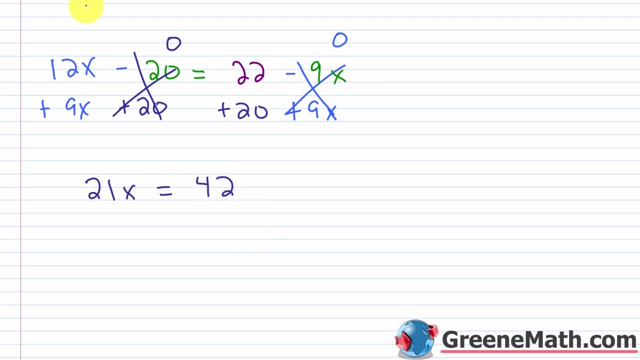 plus twenty, which is forty-two. So one last step here. to solve this, I want to isolate x. So I divide both sides of the equation by twenty-one. the coefficient of x. What's going to happen is this will cancel with this and give me an x, And then forty-two. 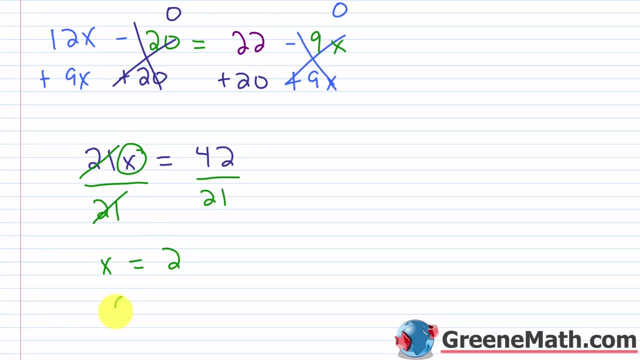 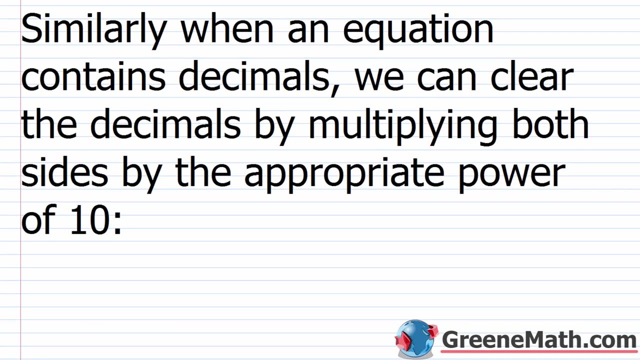 over twenty-one is two. So my solution set here contains one element, just the number two. Alright, so now let's move on and talk about equations when there's decimals involved. So I have here that. similarly, when an equation contains decimals, 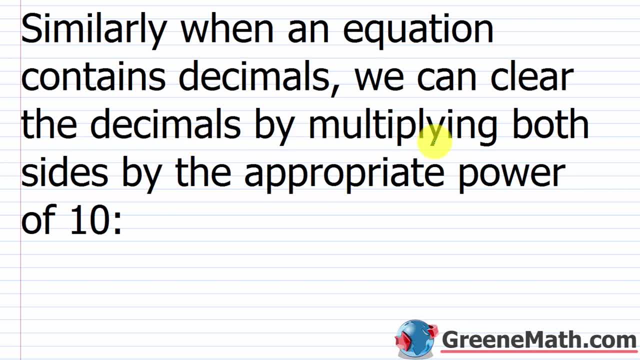 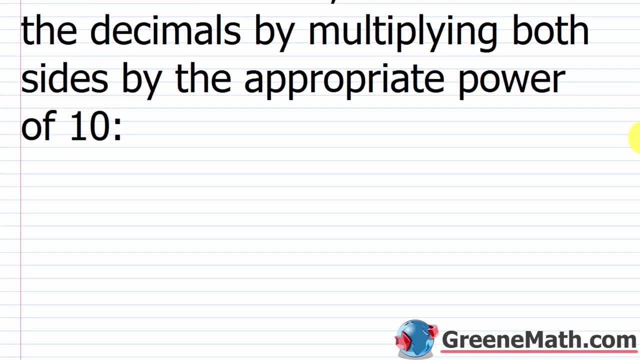 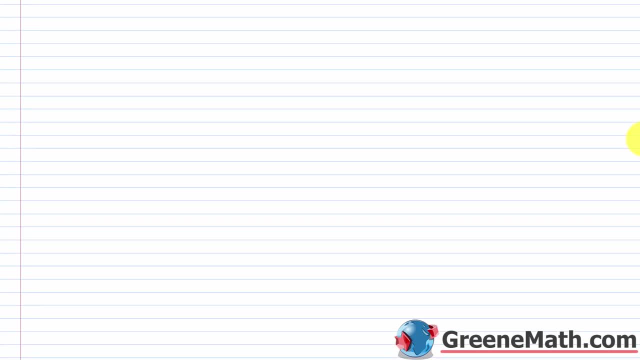 we can clear the decimals by multiplying both sides by the appropriate power of ten. So what does that mean? Well, back in pre-algebra we learned that if you multiply by ten or a power of ten, meaning something like ten to the second power, ten to the third power, ten to the fourth power. 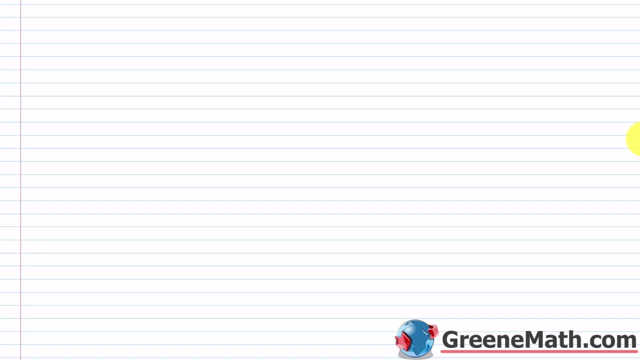 you know, so on and so forth, you're going to move your decimal point one place to the right for each zero in that power of ten. So if I have something like three times ten, we all know this is thirty. But really what I can do is I can start out with three. 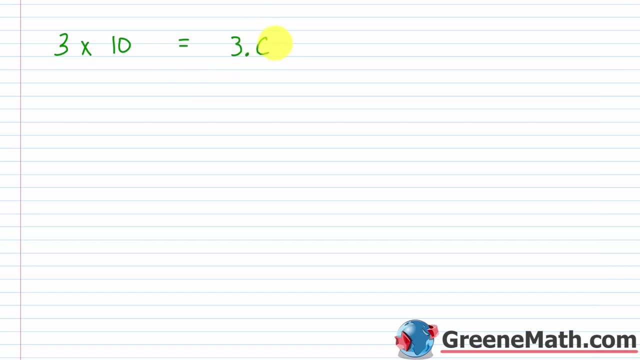 put a decimal point at the end and I can just move it one place to the right because there's one zero there. As a more advanced thing, let's say I had three times one hundred thousand, So I can start out with a three, put a visible decimal point and then I've got. 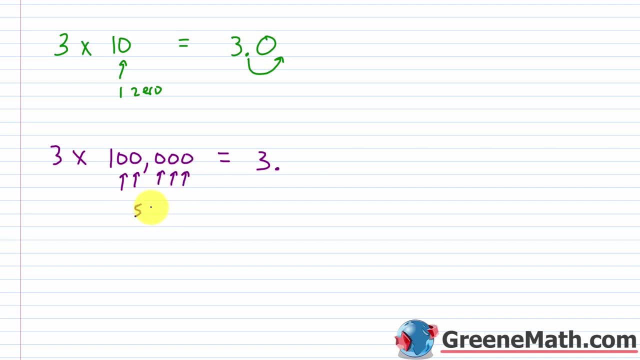 one, two, three, four, five, Five zeros. So this would go five places to the right. So one, two, three, four, five. One, two, three, four, five, And so I would have here three hundred thousand. 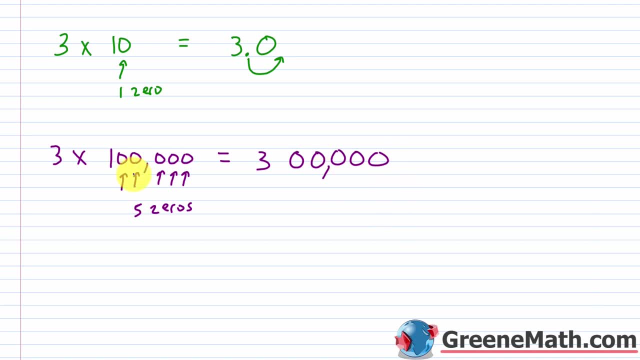 And a lot of you know that three times one hundred thousand is three hundred thousand, Just another way to kind of think about doing the operation. So when we look at equations with decimals, I just need to look for the largest number of decimal places and then our power of. 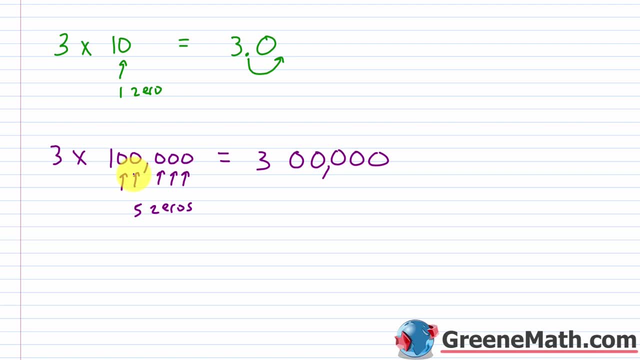 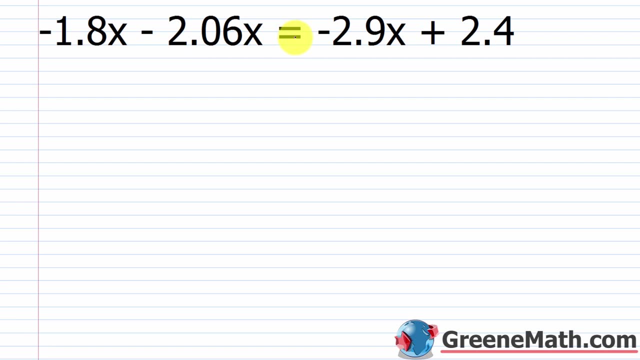 ten is going to need that number of zeros. So it's just that simple. So here's an example: We have negative one point eight x minus two point zero. six x equals negative two point nine x plus two point four. So if you want to clear the equation of decimals, and again, 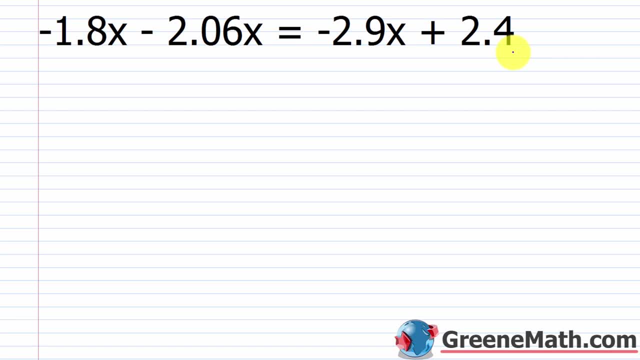 this is something that you don't have to do, it's optional. You look for how many decimal places each number is going to have. So this one has one, This one has two, This one has one and this one has one. So if I want to clear the decimals, 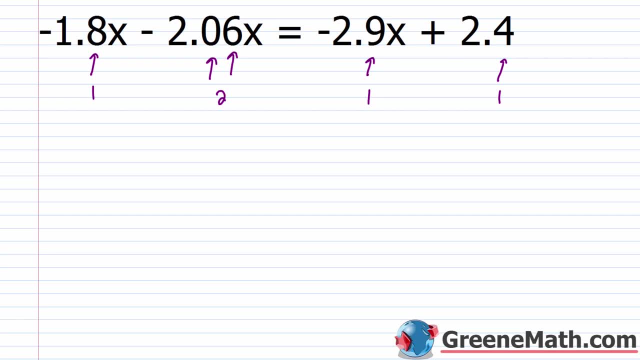 from this equation I've got to focus on clearing with regard to the largest number of decimal places. So that occurs here In this number, This negative two point zero six. So if I take care of this one, I take care of the rest. So what power? 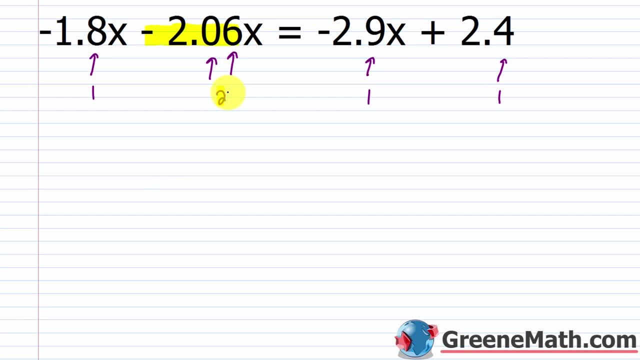 of ten has two zeros. Well, that's a one followed by two zeros or a hundred. So if I multiply both sides of the equation by a hundred, I'd have a hundred times, inside of parentheses, negative. one point eight x minus two point zero six x is equal. 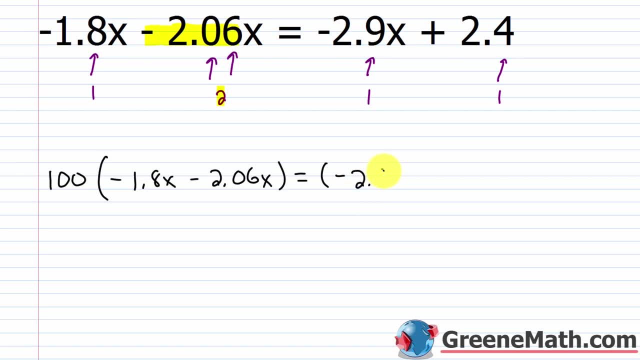 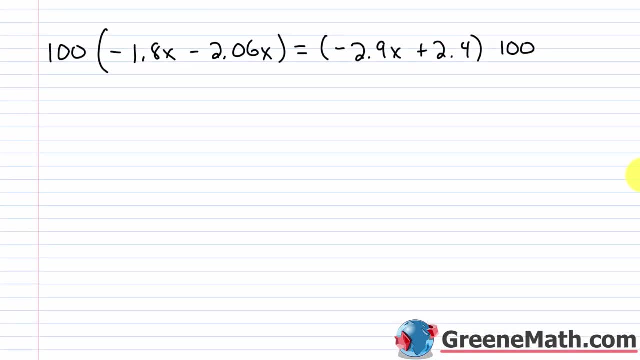 to over here inside of parentheses: negative two point nine x plus two point four, And again this is times one hundred. Let me scroll down a little bit So I use my distributive property: One hundred times negative one point eight x. So let me just write this out: 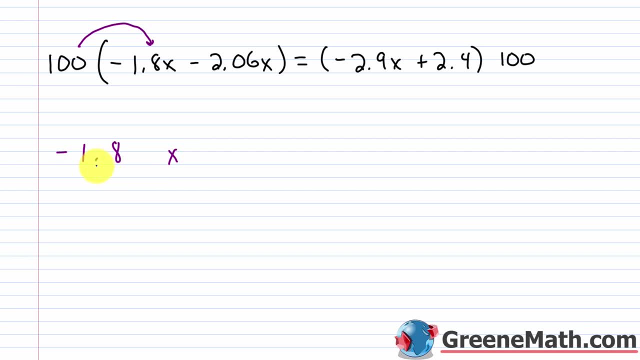 Negative one point eight x. So this is going to move one, two places to the right. This is going to be negative one hundred eighty x, Then minus. I'm going to do one hundred times this And again, I'm just moving this two. 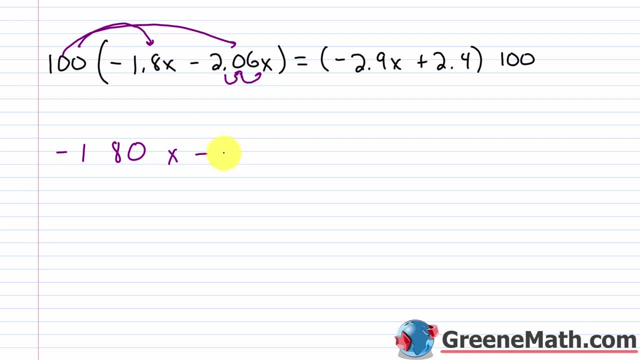 places to the right. So this and then this. So I'd have minus two hundred six x, And this equals one hundred times this, So negative two hundred ninety x. Then plus Again, I have this hundred times this, So two hundred forty. Now I've cleared the equation of decimals. 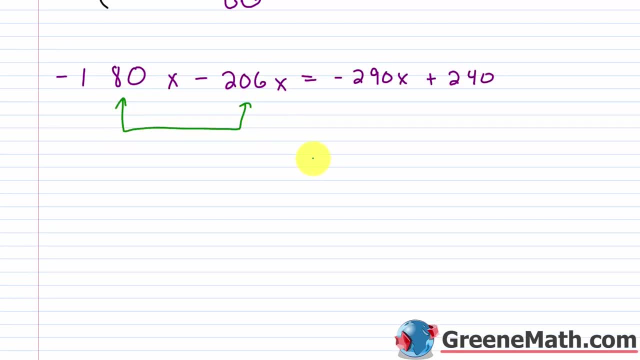 So now let me simplify over here. And negative one hundred eighty x minus two hundred six x is negative three hundred eighty six x And this equals. over here I have negative two hundred ninety x plus two hundred forty. Now let me move all the variable. 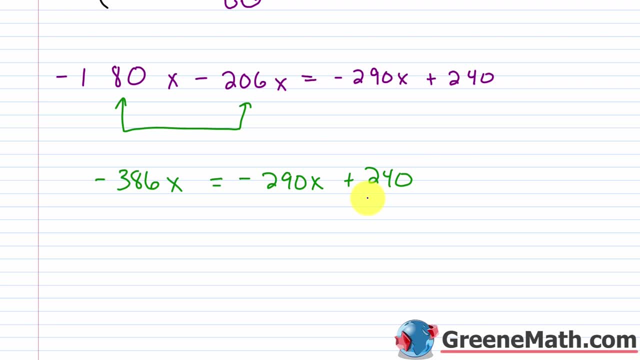 terms to one side, all the numbers on the other. So let me add two hundred ninety x to each side of the equation. So this is going to cancel. I'm going to scroll down a little bit And then negative three hundred eighty six x. 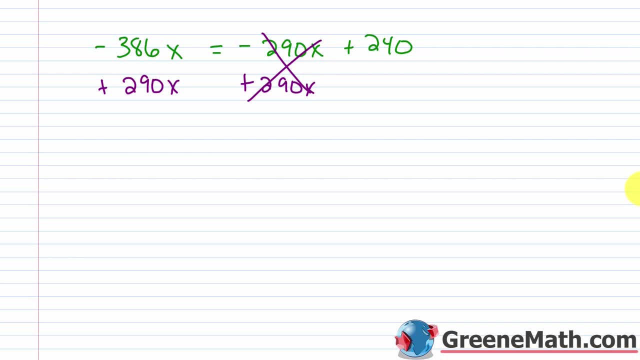 plus two hundred ninety x is negative ninety six x, So this is negative ninety six x is equal to two hundred forty, And at this point we know what to do. right, We have negative ninety six. that is the coefficient for x, So I divide both. 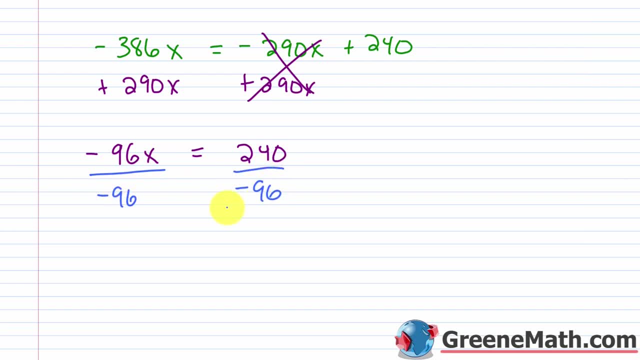 sides of the equation by negative ninety six And we'll get x is equal to: if you punch that up on a calculator, you get negative two point five. Now here's my rule of thumb: If I have an equation that has decimals involved, I use 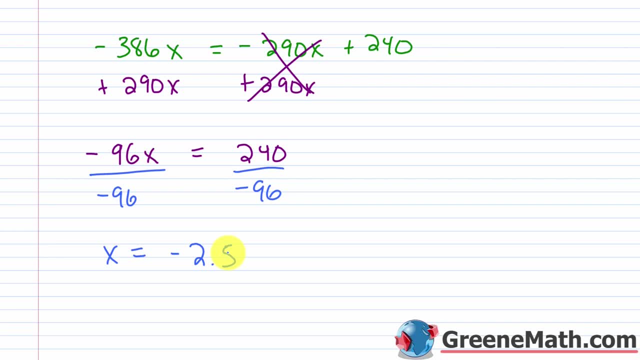 decimals as my answer. If I have an equation with fractions, I use fractions as my answer, Unless I get an integer or a whole number. In this case, it would not be incorrect to simplify the fraction and end up with negative five halves. So if I wanted to, I could factor. 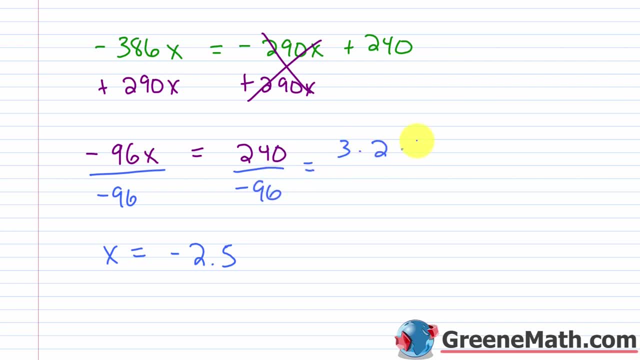 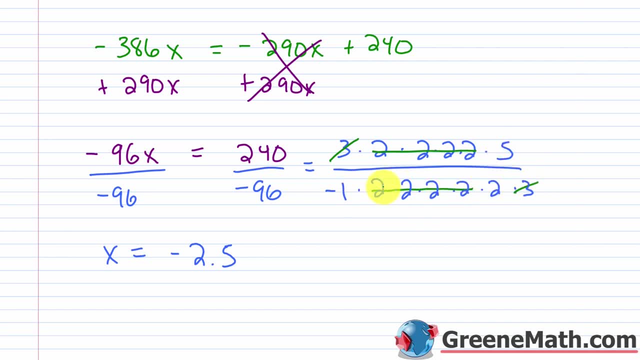 are going to cancel And I'll be left with five over negative one times two or negative five halves. So either way you want to report, your answer is okay. Negative five halves or negative two point five- It's the same value in the end. So my solution: 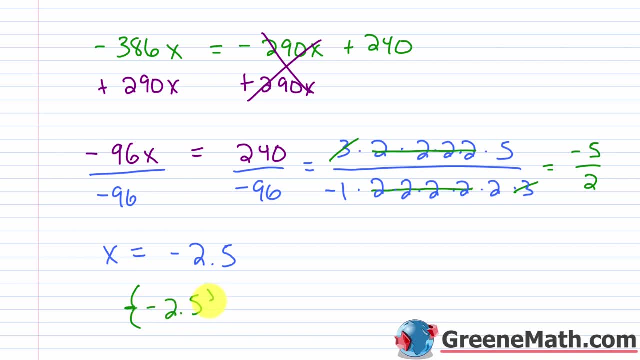 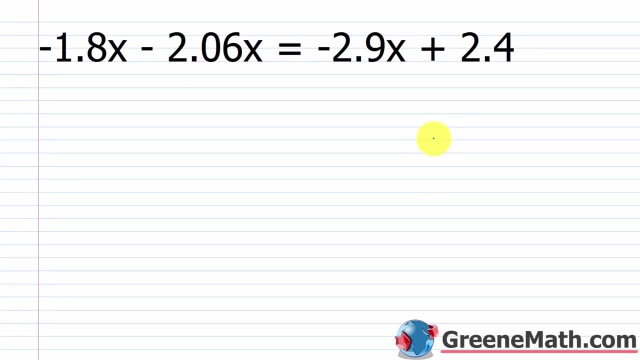 set here. I'm going to put negative two point five in And again right now I'm going to go back and show you that you get the same answer if you work with the decimals and you don't clear it. Alright, so remember, we have that x. 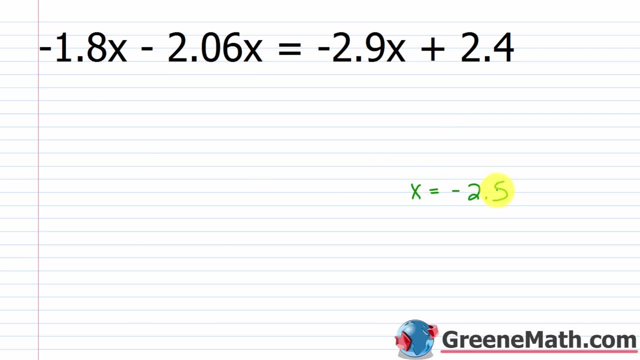 is equal to negative two point five, Or again it could be negative five halves, doesn't matter. So working with the decimals here, if I have negative one point eight x minus two point zero six x, you would end up with negative three point eight six. 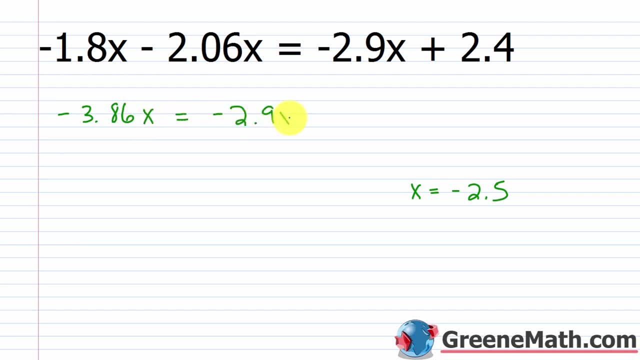 x And this equals negative. two point nine x plus two point four. I would add two point nine x to each side of the equation, So that cancels So over here. on the right I just have two point four. On the left I'm going to have negative. 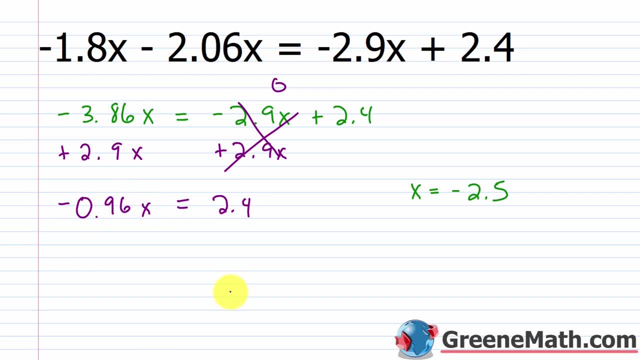 zero point nine six x. And then I want x by itself. So I'm just going to divide both sides of the equation by negative zero point nine six, And what I'm going to get is that x is equal to negative two point five, Just as I saw over here. 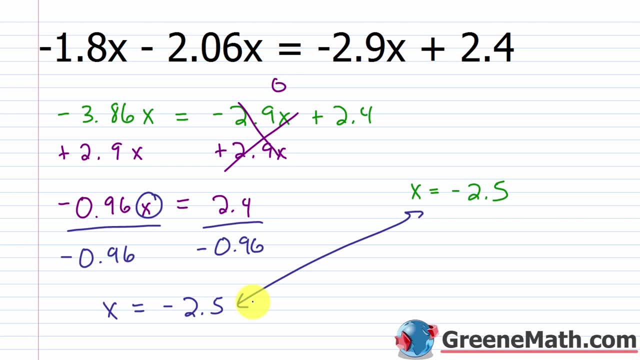 Now you might say: man, that was really quick. Why would I ever clear an equation of decimals? I would agree with you on that, But I'm teaching it because it does come up in your textbook. You might have to show your work And you need to fundamentally understand. 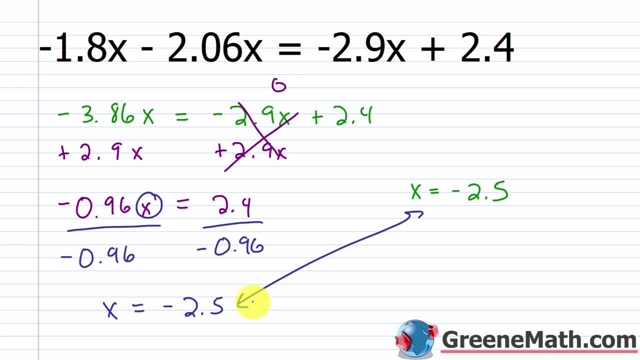 what's going on when you get a section like that in your class. But generally speaking, if you're using a calculator, it is a complete waste of time to clear an equation of decimals. I can't think of any scenario where it's going to benefit. In a lot of cases with fractions it does make it. 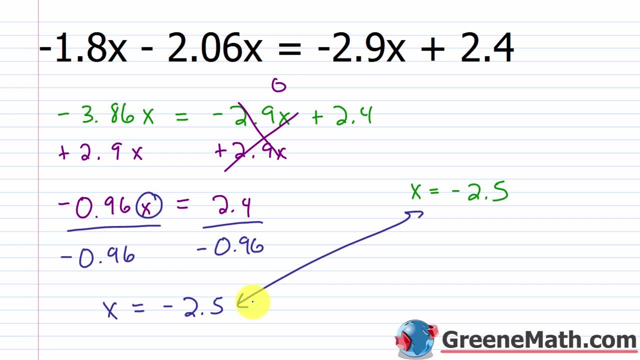 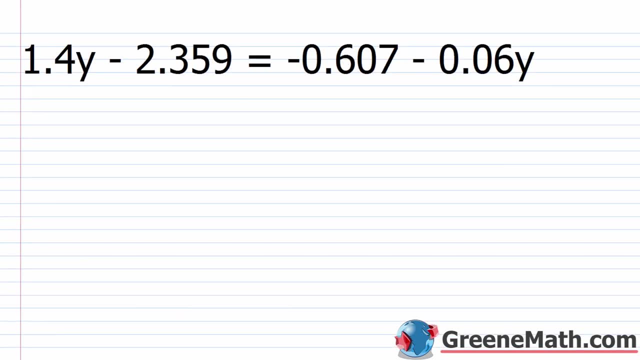 just easier if you clear the equation of fractions, But with decimals in most cases it's not really a productive activity. Alright, let's take a look at another example. So I have one point four, y minus two, point three, five, nine, And this is equal to negative zero. point six: 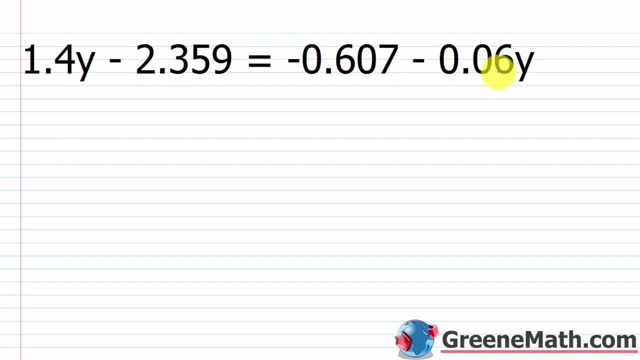 zero seven minus zero point zero six y. Alright, so I have one decimal place here, I have one, two, three decimal places here: One, two, three decimal places here And I have two here. So the highest number of decimal places occurs here and here, with three. 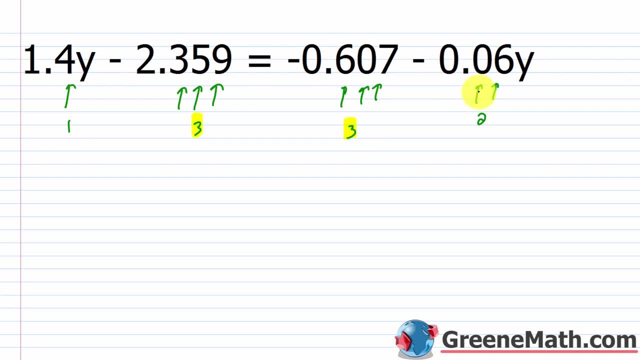 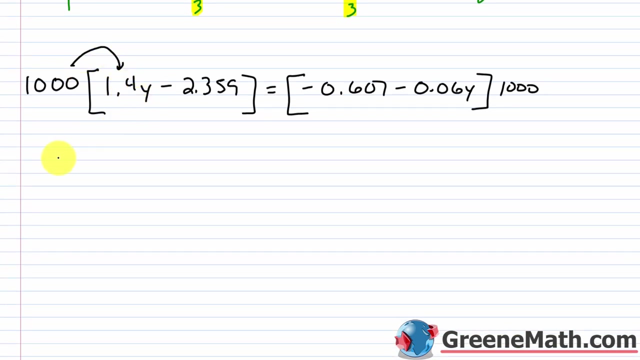 So the power of ten necessary to clear the decimals from this equation would be a one, followed by one, two, three zeros, or the number one thousand. So I multiply one thousand by both sides of the equation. Okay, so I'm going to multiply one thousand times one. point four And again the 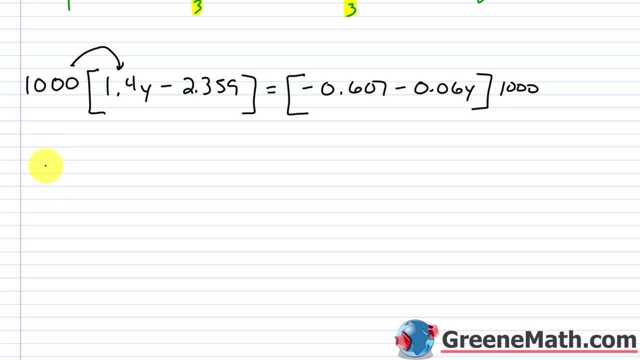 decimal point is going to move three places to the right, So that would be a one, a four, And I would have two zeros behind the four, So that would be one thousand four hundred, and then y, Then minus, if I do one thousand times two. point three: 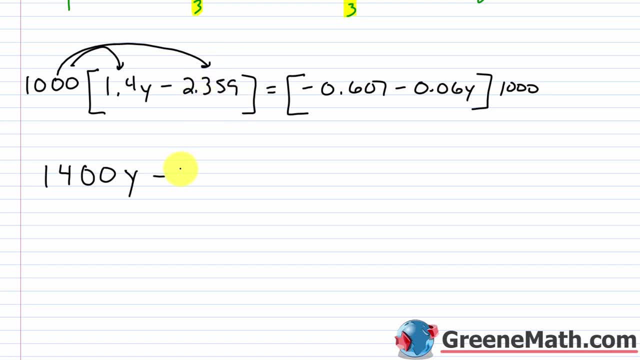 five nine. This is going to move three places to the right And I have two thousand three hundred fifty nine And this equals, if I do one thousand times this negative zero point six, zero seven. This is going to move one, two, three places to the right. 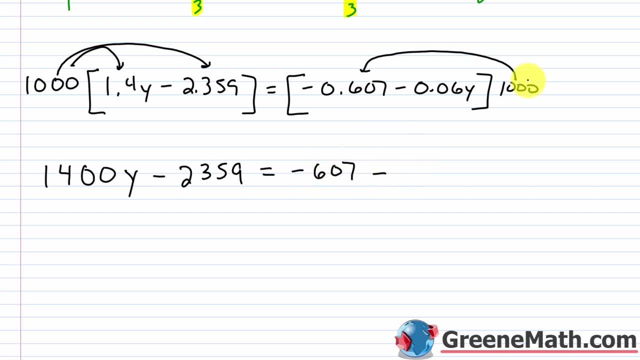 And I'll have negative six hundred seven And then minus. if I do a thousand times zero point zero, six y. I would have one, two and then a third time after that. So basically let me write this out because it's a little confusing. 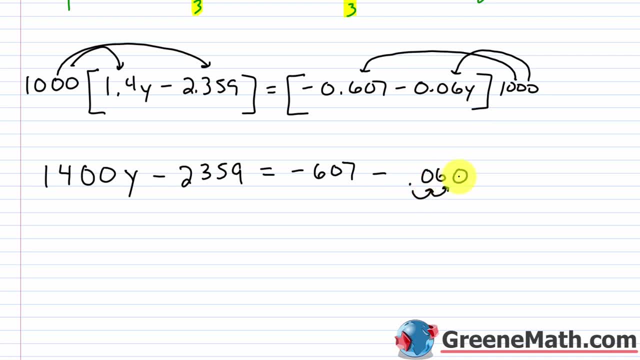 So point zero, six, this would go one, two, put a zero at the end three times, you'd end up with the number sixty. So minus sixty and then times y, Okay. so now that we have that, nothing I can do to simplify. 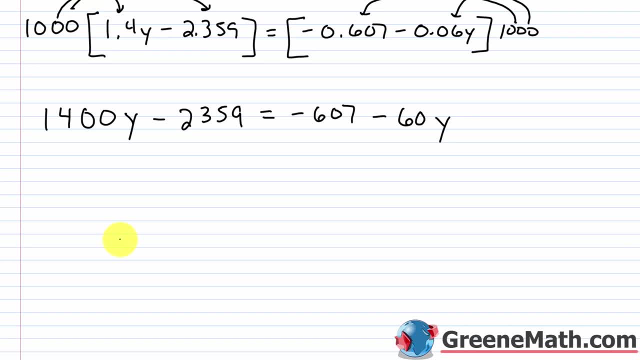 on each side. I want to move all the variable terms to one side, all the numbers to the other. So let's add sixty y to each side of the equation. That's going to cancel. And let's add two thousand three hundred fifty nine. 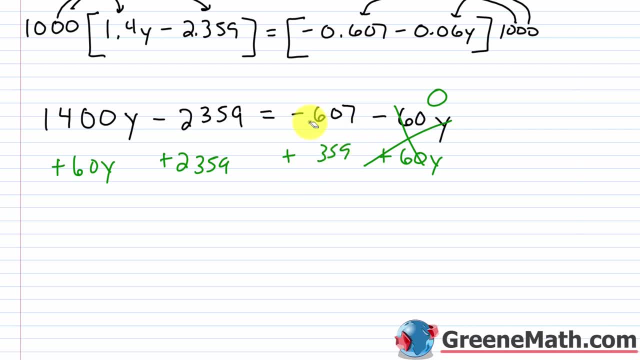 to each side of the equation. That's going to cancel. So what I'm going to have on the left side is one thousand four hundred sixty y, And this is equal to negative. six hundred seven plus two thousand three hundred fifty nine is one thousand. 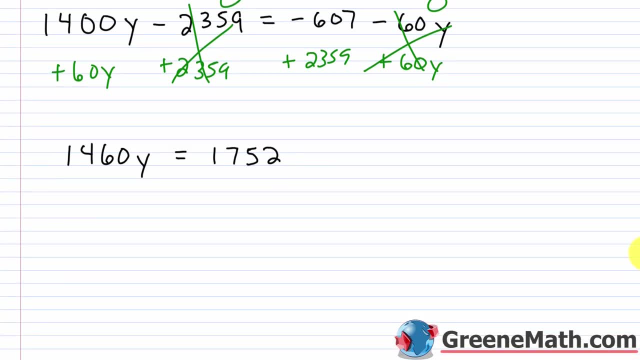 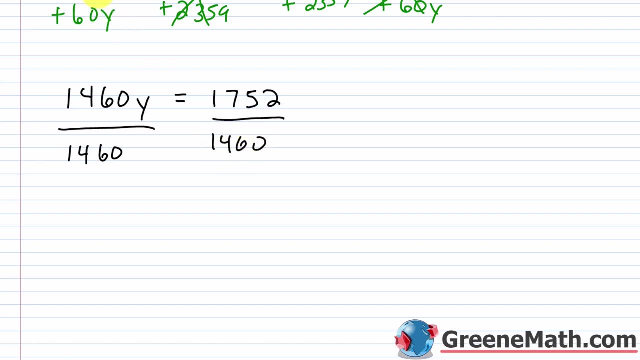 seven hundred fifty two. So the last thing to do here is to divide both sides of the equation by one thousand four hundred sixty, and this will cancel with this. On the left I just have y, and this equals, If you punch up one thousand seven hundred fifty two divided by one thousand four hundred sixty on a calculator. 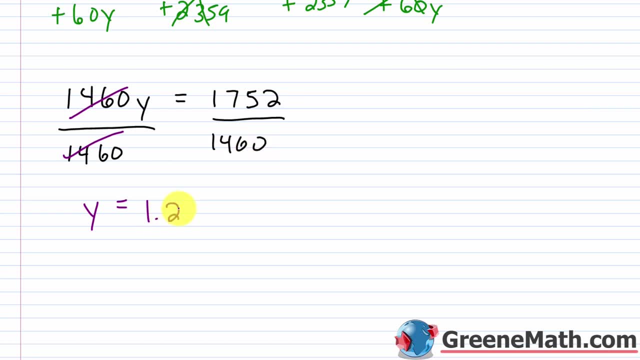 you'll get one point two. So y here equals one point two. Again, in solution set notation, inside my set braces, I just list one element, which is one point two. Alright, so the last thing I want to talk about today: when you're working with a linear equation, 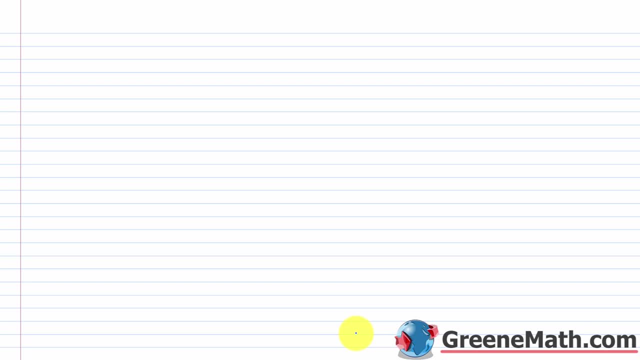 in one variable. you have three different types of equations that you're going to encounter. Now, most of the time, you're going to work with something known as a conditional equation. This is an equation that has exactly one solution. So let me just write this. 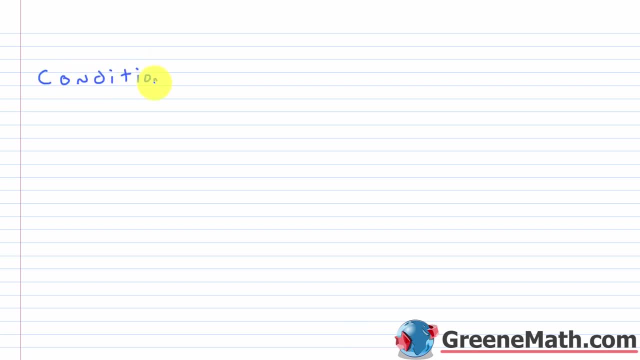 down Conditional, And this has exactly one solution. So everything we've seen up to this point has been a conditional equation. As an example, let's say we looked at five x plus one equals thirty one. This has a solution of x equals six, Because if I plug a six in for x, 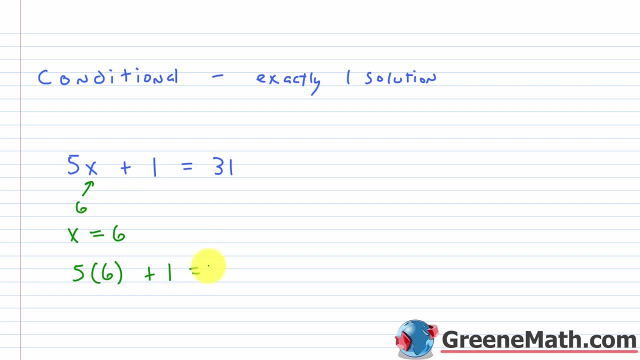 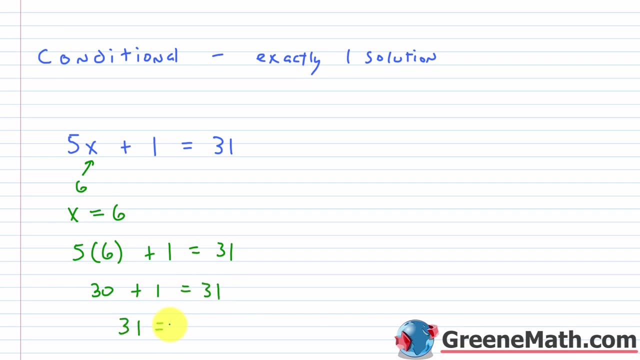 I would get: five times six plus one equals thirty one. Five times six is thirty, so you get thirty plus one equals thirty one, And then thirty one equals thirty one. Same value on the left as on the right. If I plug anything other than six in for x, you're not going to get a true statement. 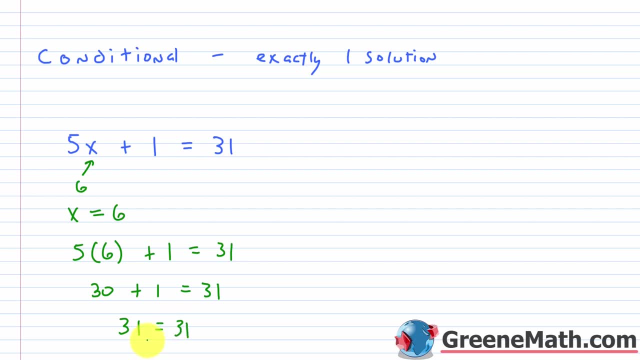 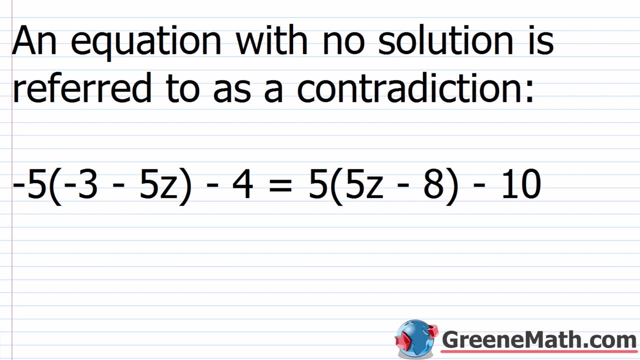 at the end, You'll have some number equals some other number, and that would be false. So conditional equations have exactly one solution, Alright. so the next situation we want to talk about is when we have an equation with no solution. So we have here that an equation with no solution is. 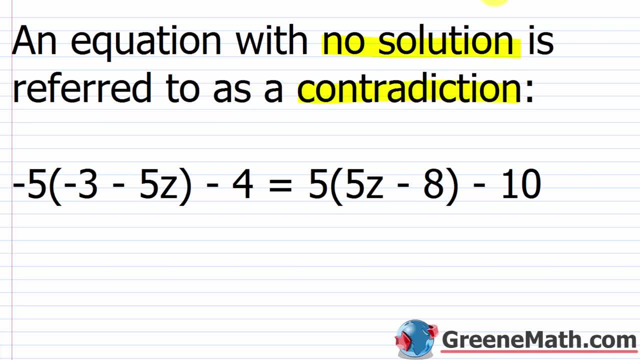 referred to as a contradiction. So I have an example of one of these and they're very easy to spot. So if you look at this guy over here, if we go to this equation, we have negative five times the quantity, negative three minus five z. then 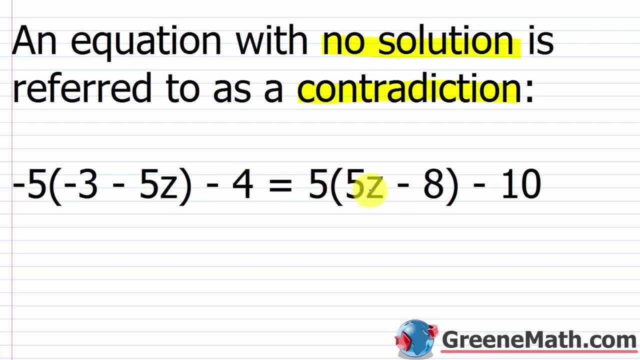 minus four. Now this is equal to five times the quantity five z minus eight, then minus ten. So we'll see what's going to happen here. is we're going to end up with some nonsense? You'll see what I mean by that. So if I use my distributive property to start, 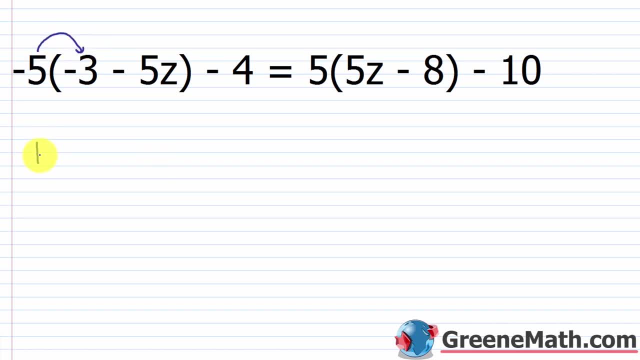 over here. negative five times negative three is positive fifteen. Then negative five multiplied by negative five z would be positive twenty five z. Now we're done with that. we just have this minus four here. so minus four, and then this equals on the right side. I'm going to use my distributive property. so five times five z is twenty five z. 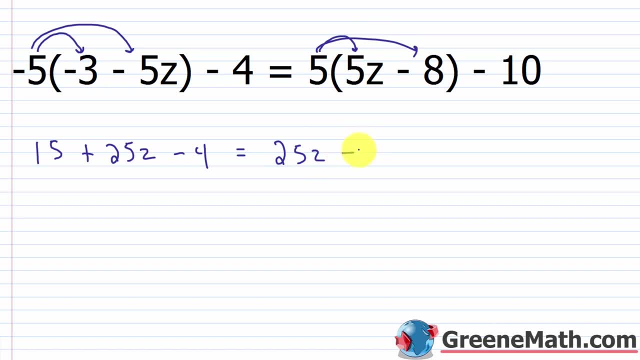 Then we have five times negative eight. that's minus forty. Then we have minus ten. So let's continue to simplify on each side. So fifteen minus four is eleven. So this side is basically twenty five z plus eleven. Then this equals. on this side we have: 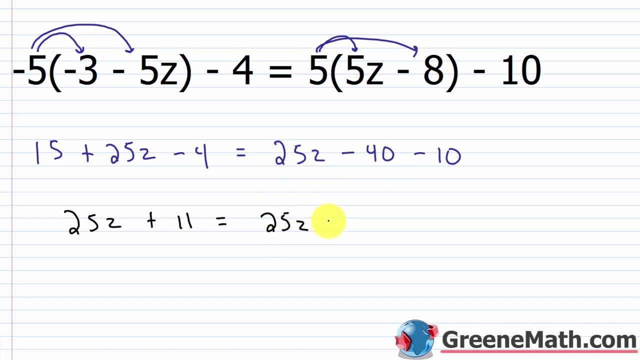 twenty five z and we have negative forty minus ten, that's negative fifty. Now, what do you see here? If you were to pause the video and really think about why you don't have a solution, what do you see? Well, what you would see if you really thought about it is: 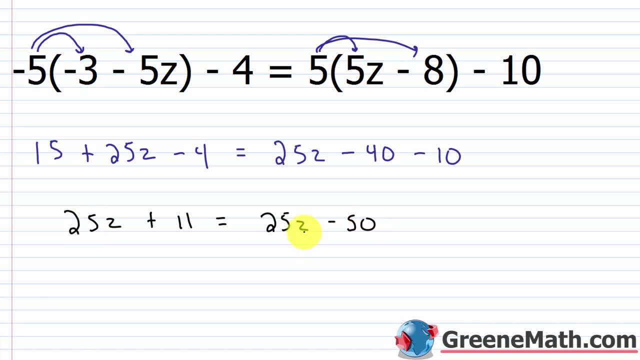 the fact that you have twenty five z here and twenty five z here. If I've got the same thing on both sides of the equation, I can just get rid of it, Because I can always go through and say: okay, minus twenty five z, minus twenty five z, subtracting the same thing from both sides of an equation. this: 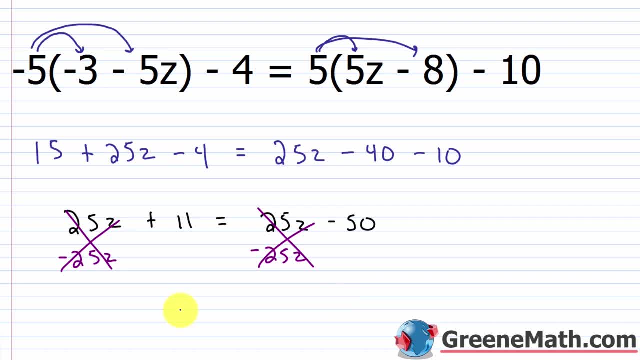 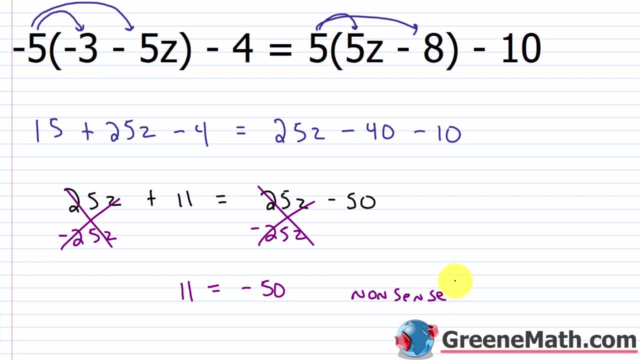 way. But where does that leave us? It leaves us with this nonsense: eleven is equal to negative fifty. Okay, let me write here: this is nonsense. Okay, This is a false statement. So your variable drops out. you're left with nonsense or a false statement, however you want to think about that. 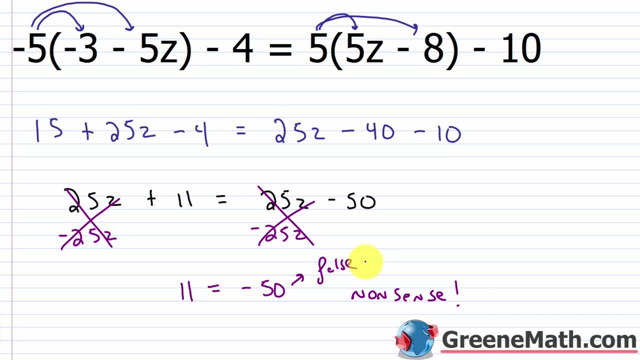 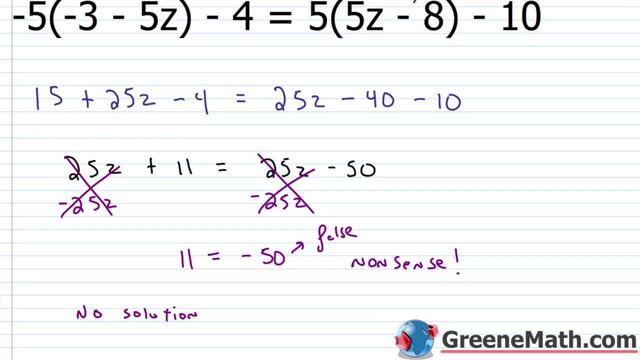 You know that you have something known as a contradiction. So if you get one of these, the way you write your answer, you can either put no solution, no solution. or if your teacher is adamant about you using solution set notation, well then you'd say that your solution set is empty. Right, it contains. 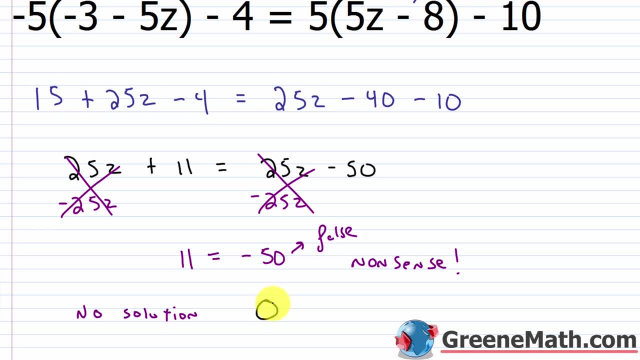 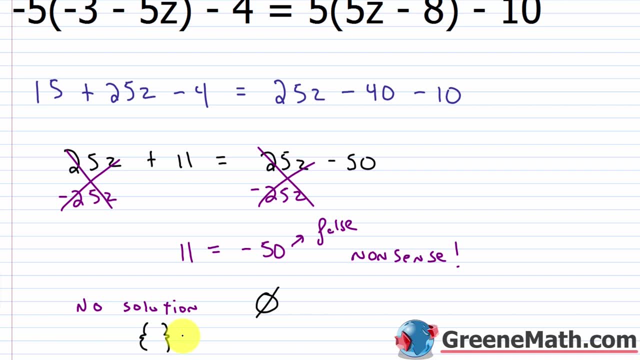 no elements. so you use the symbol for the null or empty set- Right, it looks like that? or again, you can use empty set braces. Any of these would be acceptable if you wanted to display your solution here. Alright, so the other type of equation, the last. 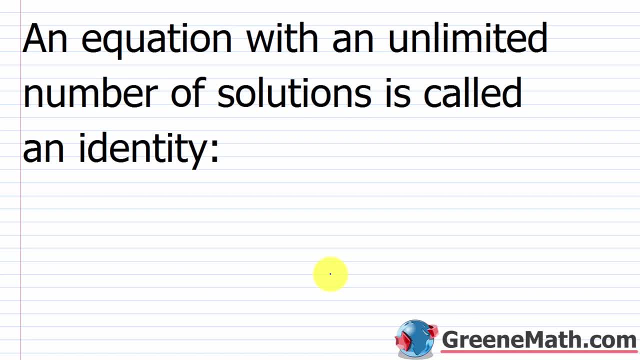 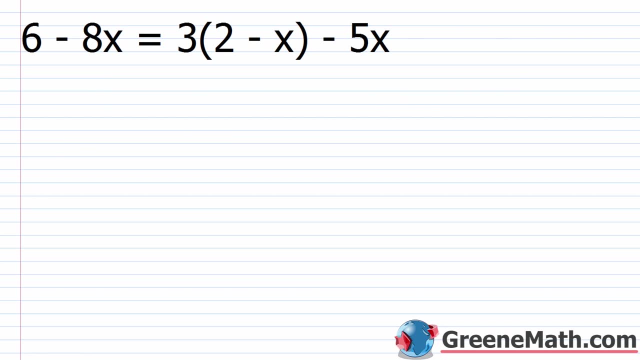 thing we would deal with is called an identity. So an equation with an unlimited- okay, unlimited, or you could say an infinite- number of solutions is called an identity. Okay, so infinitely many solutions. So here's an example of that. So let's say we're looking at six minus eight. 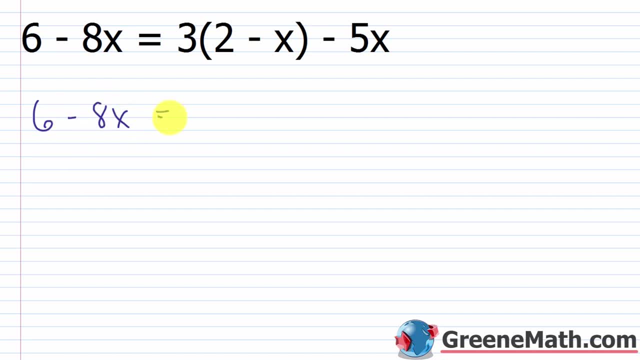 x. So six minus eight x is equal to three times two is six. Three times negative x is negative three x. And then you have minus five x, So negative three x minus five x is negative eight x. And what you basically have here is the same thing on each side of. 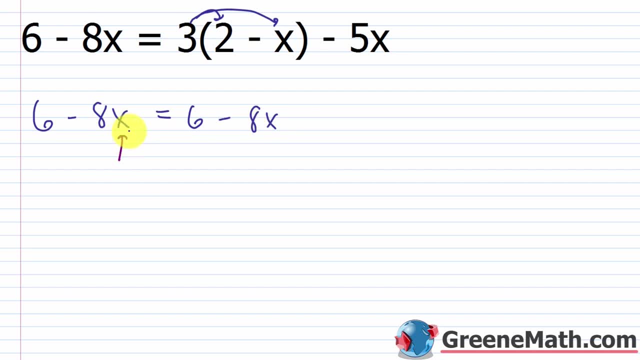 the equation. So no matter what value I choose for x, doesn't matter what it is. If I plug it in for x, I'd end up with the same amount, Right, because I'd have six minus that same amount, no matter what I choose. 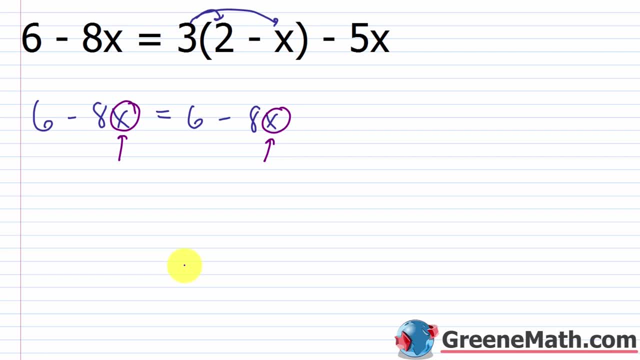 So in this particular case, if you don't catch it right away, essentially when you go to simplify, let's say I subtract six away from each side of the equation, that's gone, and that's gone. And then let's say I add eight x to each side of the equation. 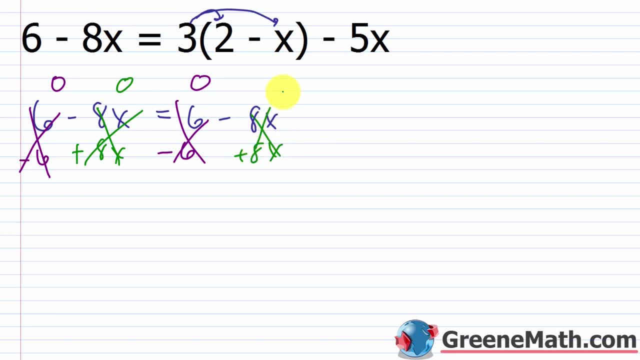 that's gone and that's gone. So you end up with zero equals zero, which is true. So you end up with a number equal to another number and the variable just drops out, Just gone. Okay, so you can just put here that there's an. 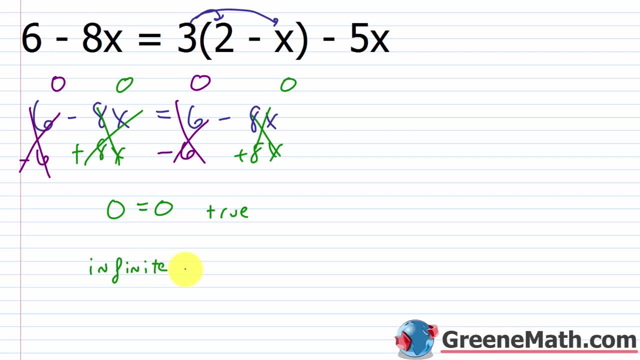 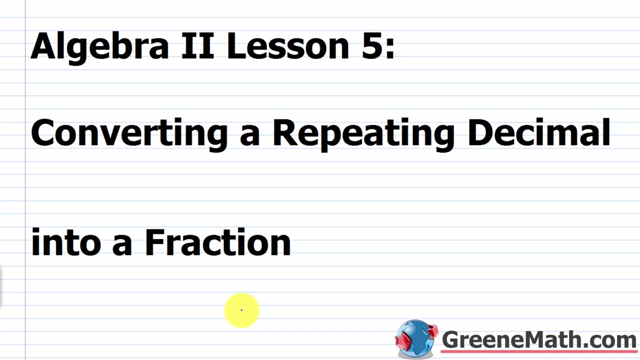 infinite number of solutions Or in solution set notation inside of set braces. you can simply write all real numbers And there's more ways to kind of notate this, but this would be the two easiest ways to write that answer on your test. Hello and welcome to Algebra 2, Lesson 5.. In this 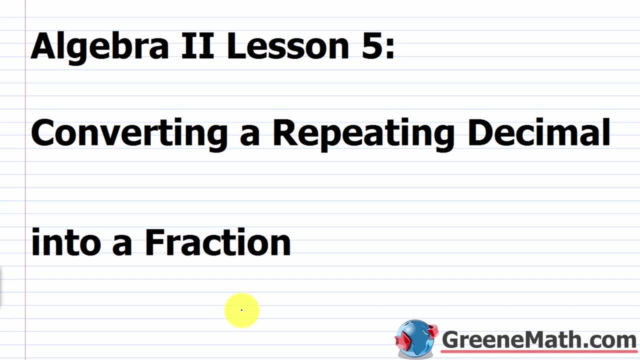 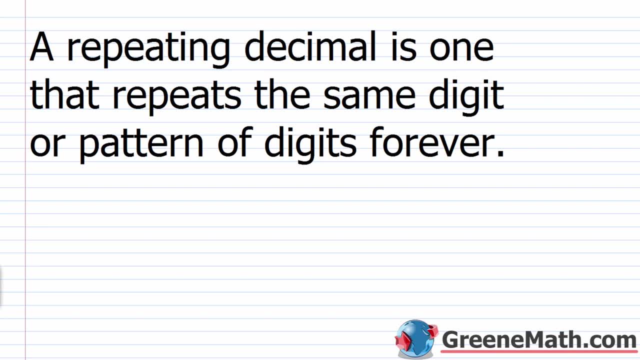 video we're going to learn about converting a repeating decimal into a fraction. So back in pre-algebra we learned how to convert back and forth between decimals and fractions, But for most of you, you were probably never shown how to convert a repeating decimal into a fraction. So we'd start out with just asking what. 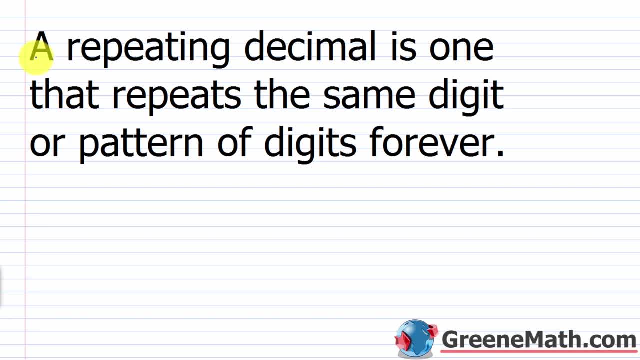 is a repeating decimal, Just in case you don't know. So a repeating decimal is one that repeats the same digit. Okay, it repeats the same digit or pattern of digits forever. So as an example, let's say you had something like 0.267777. 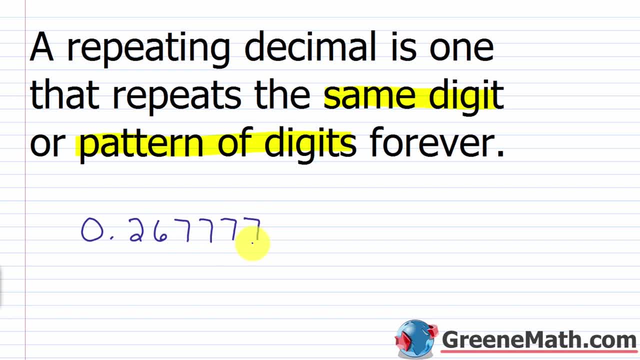 where the 7 is going to repeat forever. so we can put the three dots after this 7 here to indicate that the 7 will continue on and on and on. Another way you can notate this: you could write this as 0.267. 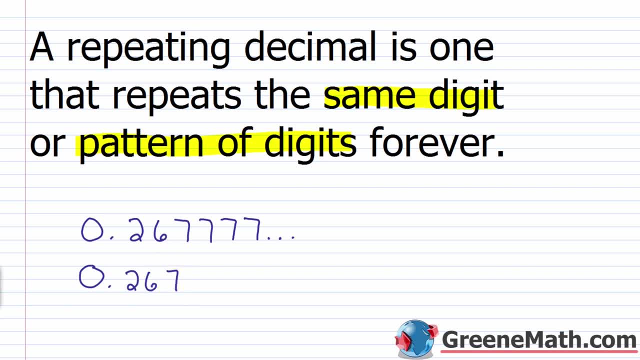 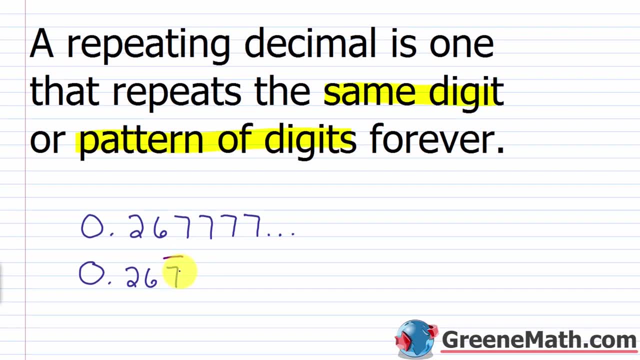 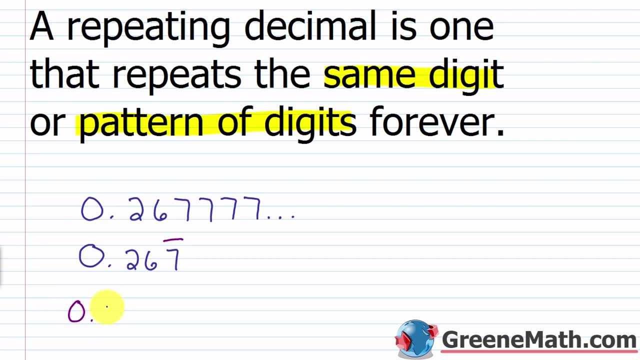 0.267 with a bar over the 7. You put a bar over the digit or series of digits that's going to repeat forever. Now, as another example of one of these, let's just look at two more. Let's say I saw something like 0.43. 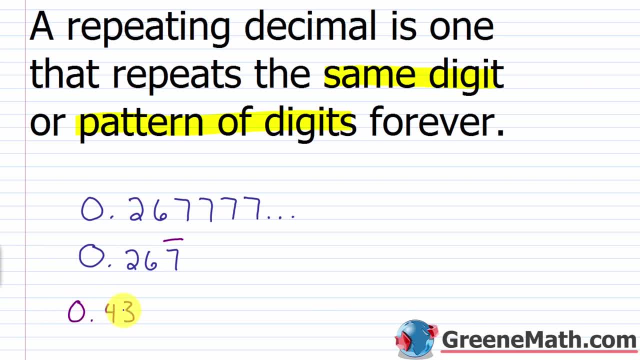 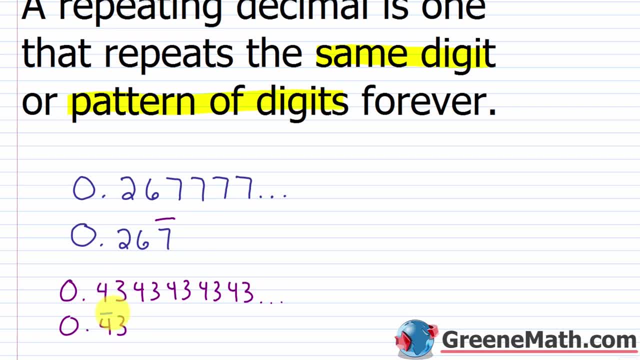 with a bar on top of the 4 and the 3, because that pattern of digits is going to repeat forever: A 4 and then a 3. A 4 and then a 3. So on and so forth. Or, as another example: 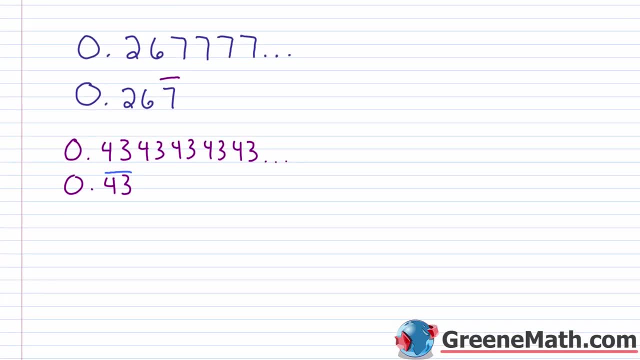 let's say I saw something that was kind of longer. Let's say I saw 0.39176, 0.39176, and let's say the 176 repeats forever. So then 176, 176, 176, you know, so on and so forth, So I can put the three dots here. 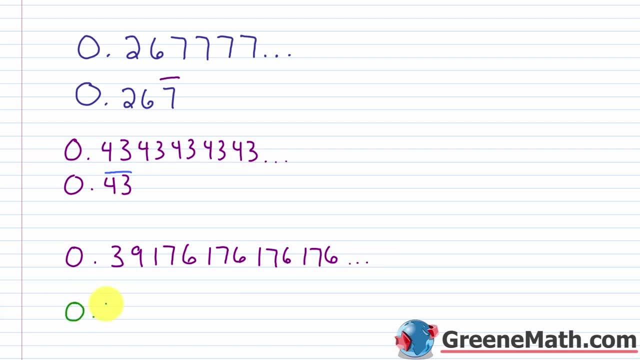 Or again I can write this as 0.39176, 0.39176. and again I can put a bar on top of the 1, the 7 and the 6. The three digits that are going to repeat forever. Okay, so let's jump into. 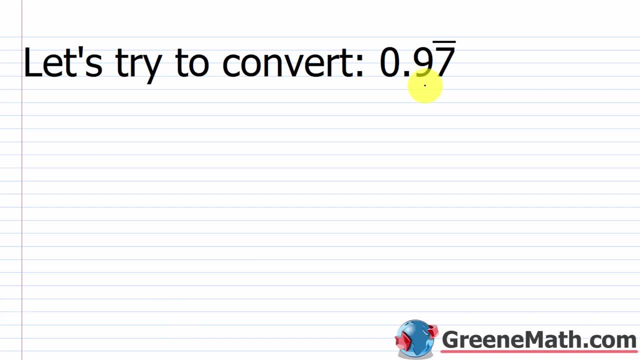 an example now And for a lot of you this is not going to be very difficult. I can tell you that you just write down the steps as we're working through these problems And once you do your own practice problems, after 5 or 10 of these, you're going to have this down pack. It's going to be 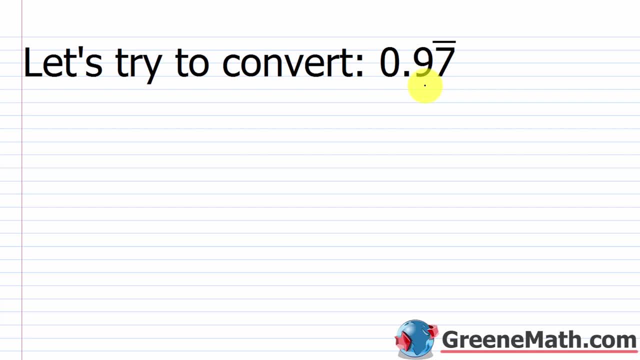 no issue for you in the future. Again, this is very, very simple. So let's try to convert 0.97, where the 7 repeats forever. Again, notice the bar on top of the 7 there. So the very first thing that you want to do is set a variable like x or y or 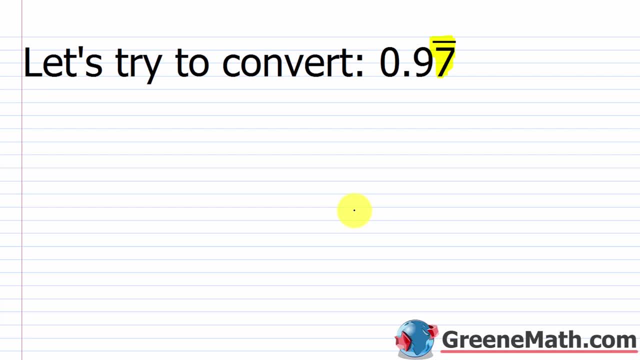 z or whatever you want to use, equal to the value Right the repeating decimal. So let's just go ahead and use x and say x is equal to 0.97, where the 7 repeats forever. And for the sake of this example I'm not going to write it like: 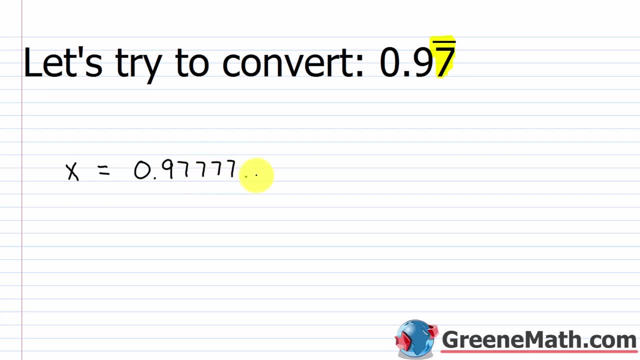 this. I'm going to write it like this, And it's just going to make it easier to see what's going on. Then the next thing I want to do: I want to multiply both sides by 10 to the power of n, And n is just going to be the number. 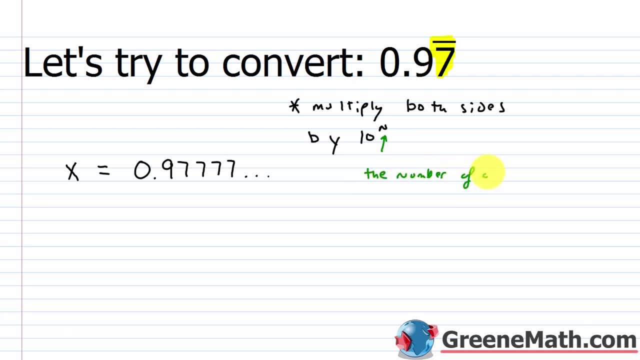 of digits in the repeating string. Now, in this particular case, I have one digit that's going to repeat forever. So 10 to the power of, in this case it would be 1.. 10 to the power of 1 is 10.. We all know that. So if I multiply both sides of the, 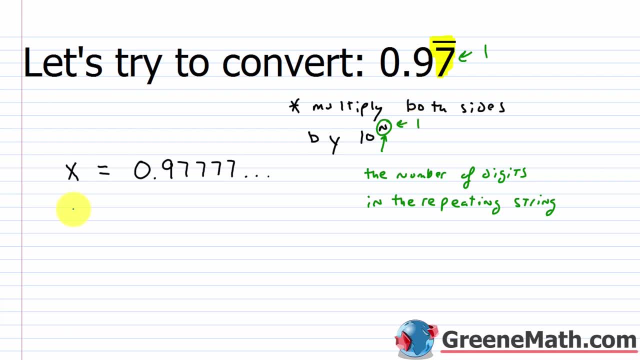 equation by 10. what am I going to get On this side? I'm going to get 10x On this side, I would move my decimal point one place to the right and I would have 9.77777.. You can write as many 7's as you want, Just making it clear that the 7 repeats forever. 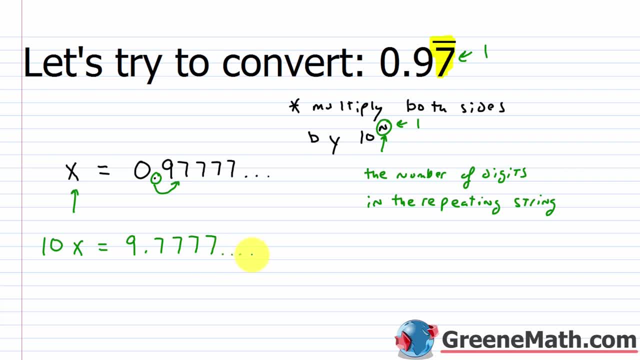 And go ahead and put your 3 dots at the end. Now, at this point, I have not gotten rid of the repeating decimal. It's still right here That 7 is still repeating forever and ever and ever. But the step we're going to do now is going to get rid of it. So what I'm going to do, 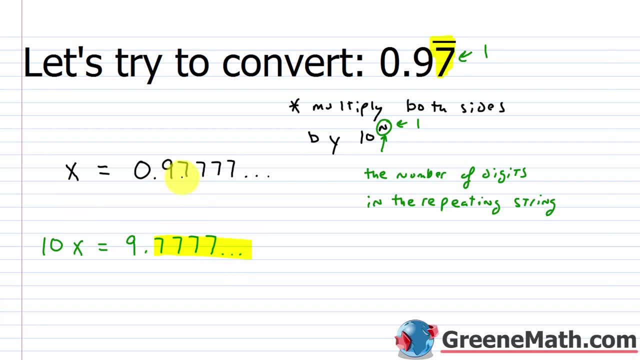 is? I'm basically going to subtract the original equation from this new equation I just got by multiplying both sides by 10.. So you might say: how is that legal? Remember, these two sides are equal to each other. On this side, I'm going to subtract. 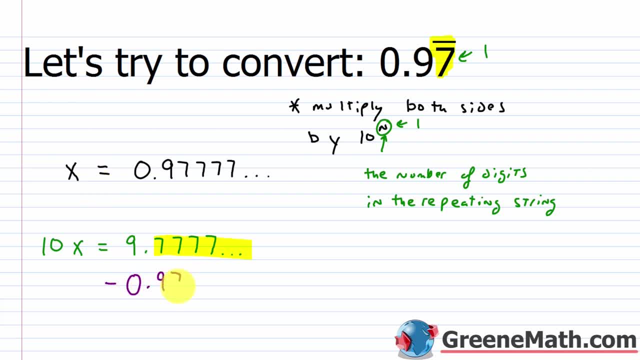 away 0.9777 with the 3 dots there. And what's going to happen is this part right here is going to go away. It's just going to cancel. 7-7 is 0.. So all this is gone And I'm left with 7-9. 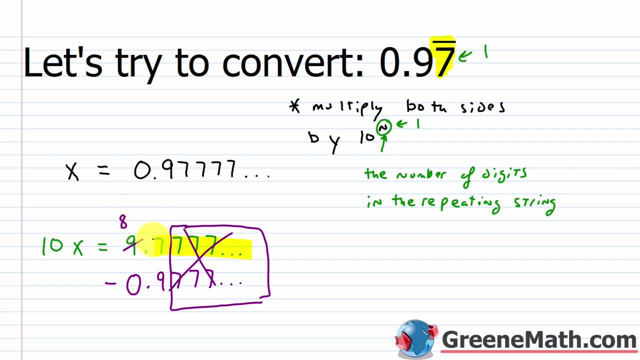 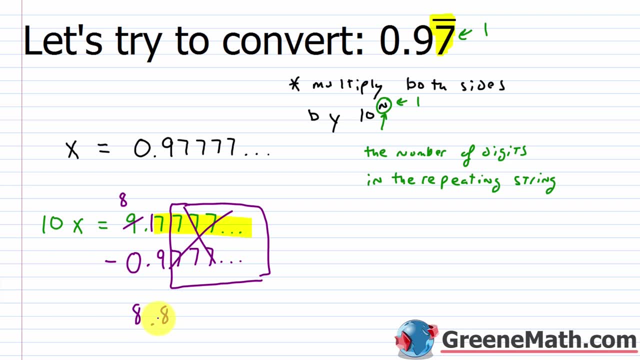 I'd have to borrow to do that. So I'd borrow from this. This would become 8.. This would become 17.. 17-9 is 8.. Put my decimal point: 8-0 is 8.. So this side is now 8.8.. 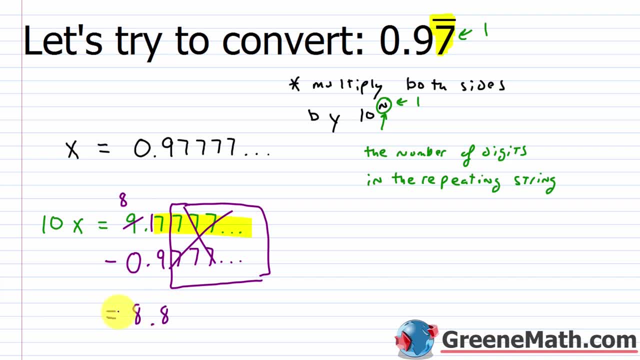 So let's put this: equals Over here I'm going to subtract away x And remember this is legal because x is equal to this value and I'm basically subtracting away the same thing from each side of the equation. So 10x minus x is going to give me 9x. Now 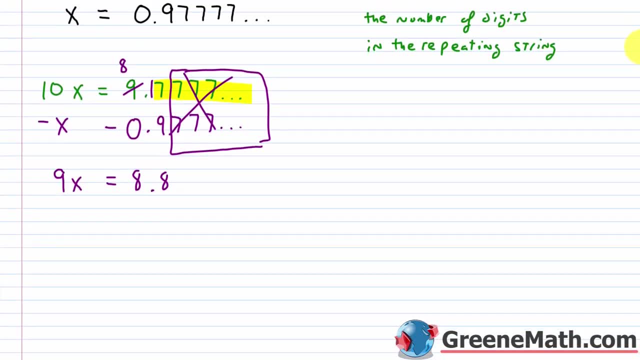 let me do one more thing here. Let me scroll down and get a little room going. I'm just going to multiply each side of the equation by 10, again to clear this decimal point. I'm going to multiply this side by 10 and this side by 10. 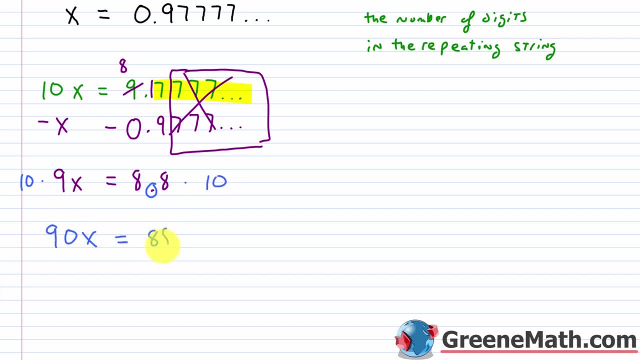 and I'm going to get that- 90x is equal to 88. This goes one place to the right. So now we have something very easy to solve. We divide both sides of the equation by 90. The coefficient of x- And this is going to cancel with this And I'm going to be left with x. 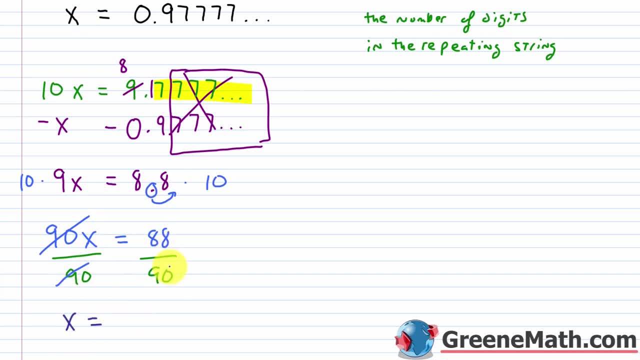 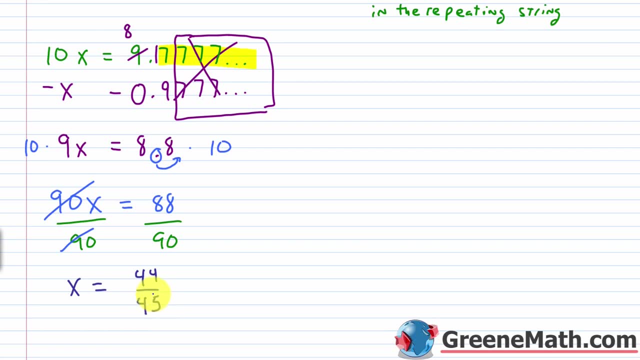 is equal to 88 over 90, which can be reduced. Each is divisible by 2.. 88 divided by 2 is 44. And 90 divided by 2 is 45. So there is your solution: x is equal to 44 over 45. And remember. 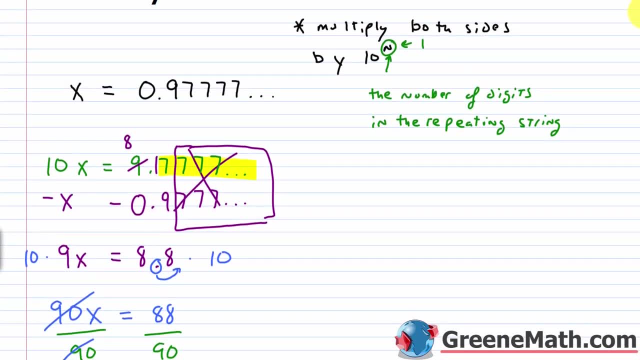 if we scroll back up here, In the beginning we said x was equal to this. So if I replace x with this value of 44 over 45, these two have to be equal. So that's your value: 44 over 45 is equal to 0.97777. 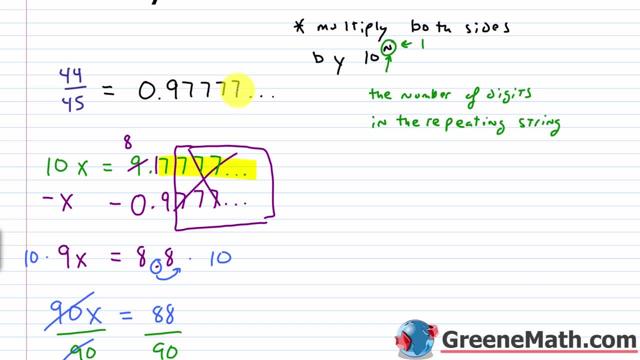 where the 7 repeats forever and ever and ever. And if you don't believe me, punch it up on a calculator. If you punch up 44 divided by 45, you will get 0.97, where the 7 repeats forever. Now your calculator will do one of two things. It may truncate. 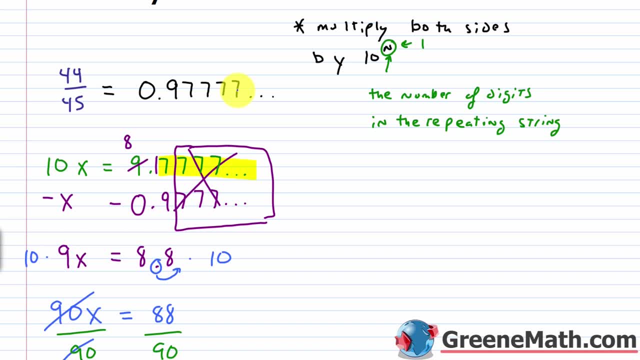 so it may stop displaying 7's. It's just not displaying anymore because it just can't, Or it may round at the end so you might see the final digit as an 8.. But that's not the actual value, That 7. 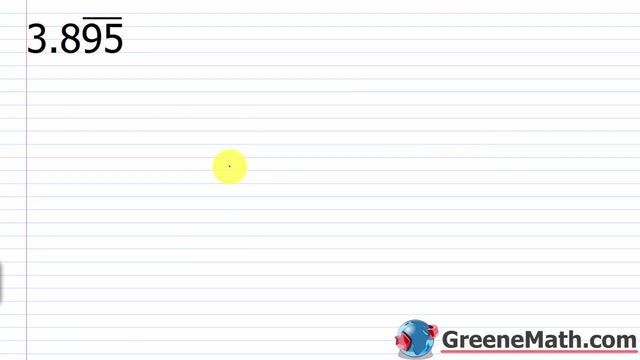 is going to repeat forever and ever and ever. Okay, so your brain might be a little fuzzy from the first one, But hopefully on the second one here you're going to catch up and kind of get in the flow of things. So we have 3.895, where the 9 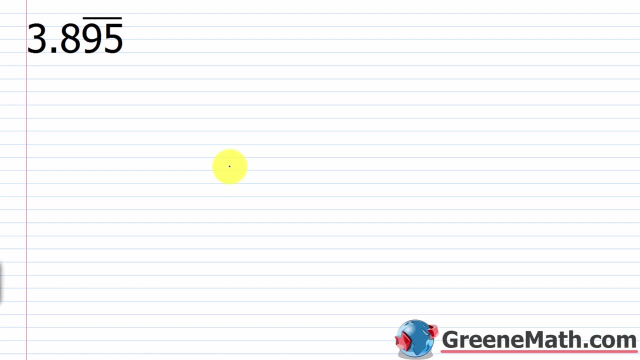 and the 5. That series of digits there is going to repeat forever. So we would see something like 3.895, 95, 95, right, so on and so forth. And again I want to set this value equal to a variable like x or y or z. 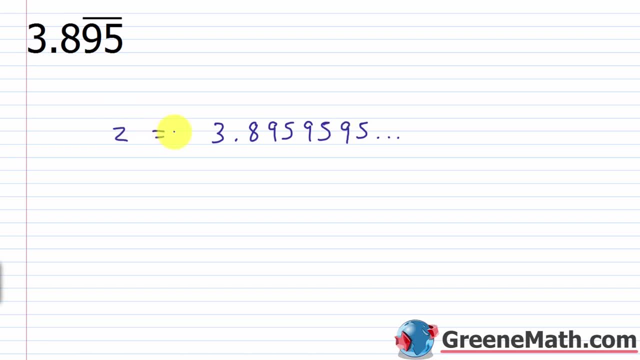 Let's go ahead and just use z, Kind of spice things up. I know we always like to use x, And then the next thing I want to do is I want to multiply both sides of the equation by 10 to the nth power, where n again is the number. 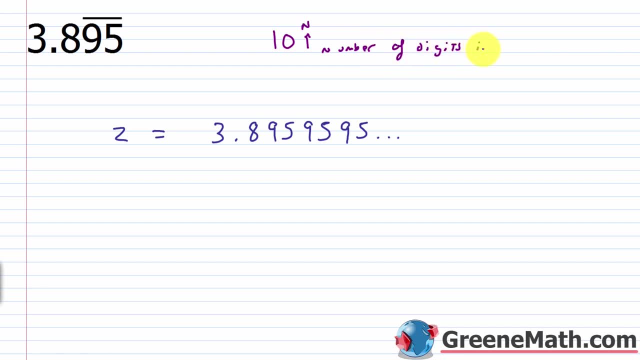 of digits in the repeating string. So in this case I have one, two digits there, So n is going to be a 2. So 10 to the second power is 100.. So one followed by two zeros. So this over here, if I multiply both sides by 100. 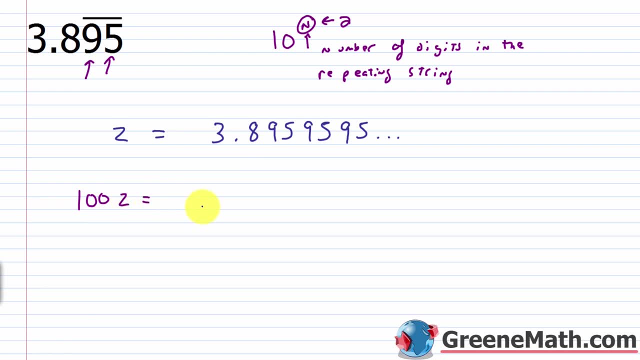 this would be 100z and this would be 389 point Right, because this is going to move two places to the right. So you'd have 389 point, and now I'd have a 5 and then I'd have my repeating digits, So I would have 95. 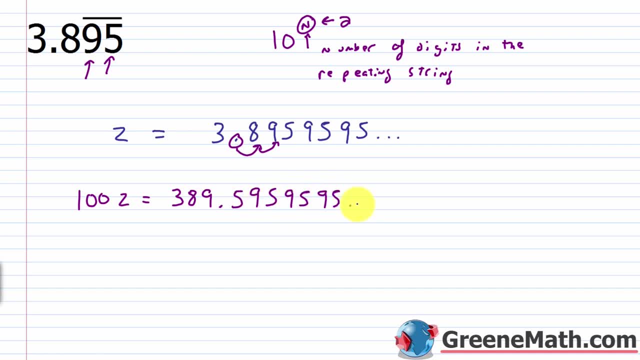 95. And I could do another one, 95, and then the three dots. Okay, so now we know that we want to subtract this value from both sides of the equation, So I'm going to subtract away 3.895, 95- 95. 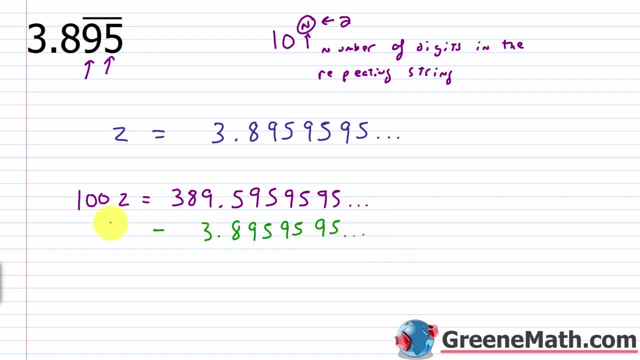 where the 95 repeats forever. And I'm going to do the same thing over here. but remember, on this side I want to subtract away z And again, that's legal because this is equal to this. So I'm subtracting away the same thing from both sides of the equation. So over here I'm going to have 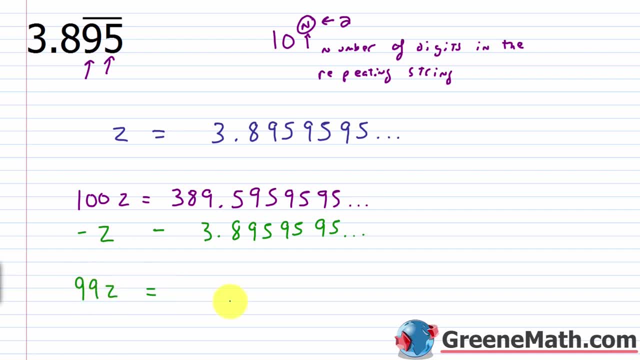 99z And over here, if I do my subtraction, I know from this point on it's going to cancel. This is going to cancel itself out. Then over here I'm going to borrow: This will become 8.. 15 minus 8 is 7.. 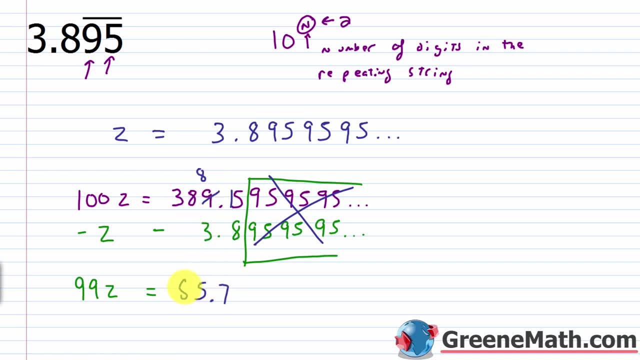 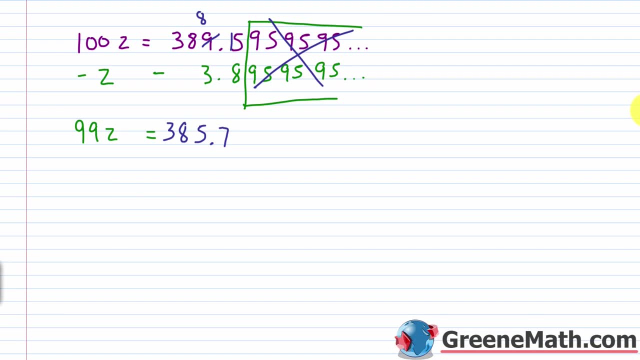 Put my decimal point, 8 minus 3 is 5.. Then I have my 8 and I have my 3.. Alright, let's scroll down and get a little room. And now let me just clear this decimal from the equation. Let me multiply both sides of the equation by 10.. 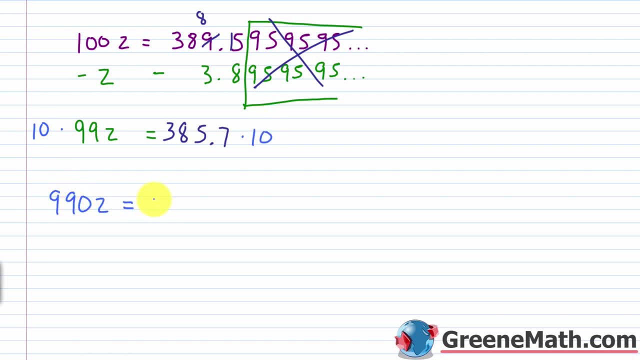 And I'm going to get: 990z is equal to 3857.. Now I want to just divide both sides of the equation by 990.. So z is by itself. Divide this by 990.. Alright, so let's write this as z is equal to. 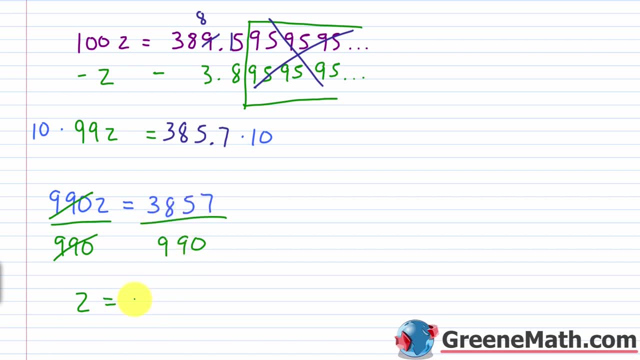 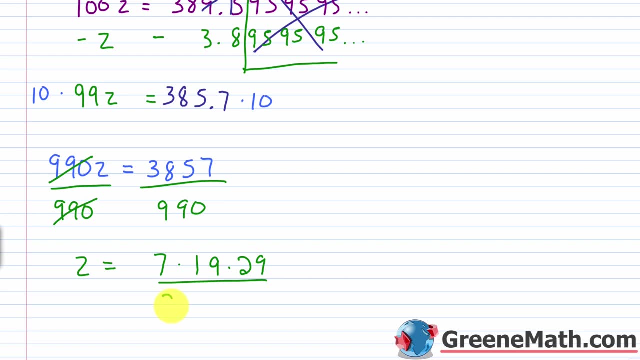 I can factor 3857 into 7 times 19 times 29.. And then I can factor 990 as 2 times 3 times 3 times 5 times 11.. So between the numerator and denominator I don't have any common factors. 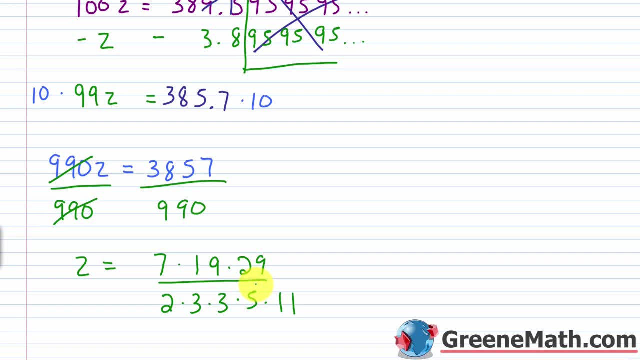 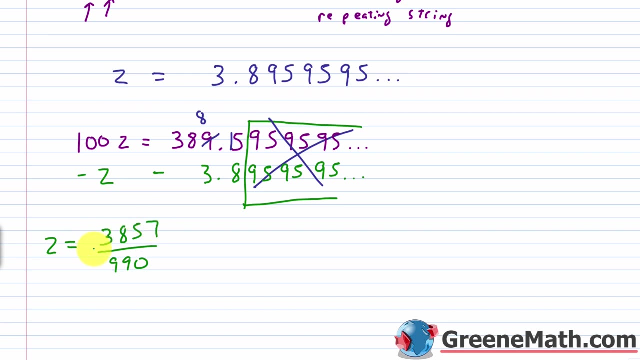 other than 1.. So there's nothing I can really do. My answer is going to be that z is equal to 3857 over 990.. And again, if we go back up, we see that z was equal to this. So I can. 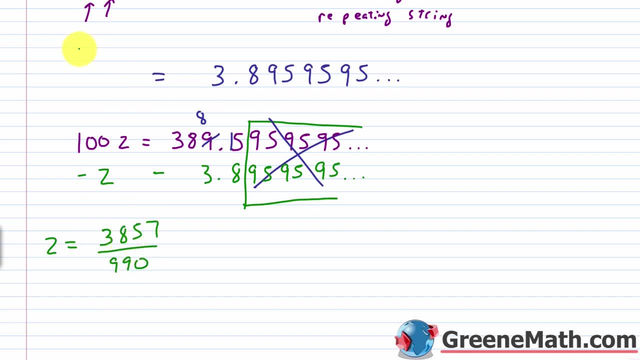 replace this side right here with this: I can say that 3857 over 990 is equal to 3.895.. And in more convenient form, I can put the bar over the 9 and the 5 to show that 95. that series of digits is going to repeat forever. 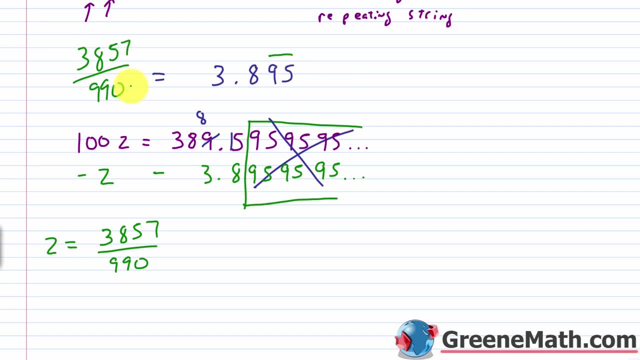 So again, punch this up on a calculator: 3857 divided by 990, and you will see this. But again, your calculator will either truncate and stop at some point with a 5, or it will round up and you'll see a 6 as. 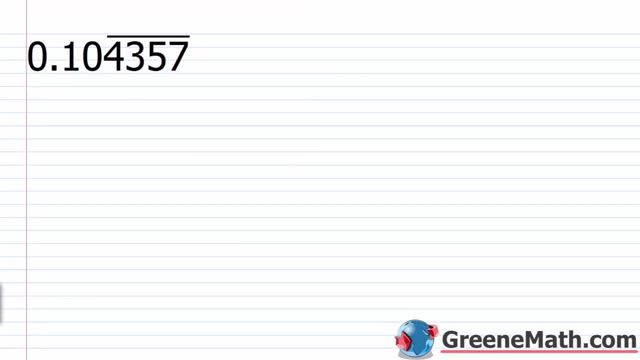 the very final digit. Alright, let's take a look at another one. So we have 0.104357, where the 4357 repeat forever and ever and ever. So again, let's assign this to a variable. Let's use y this time. So let's say y is equal to. 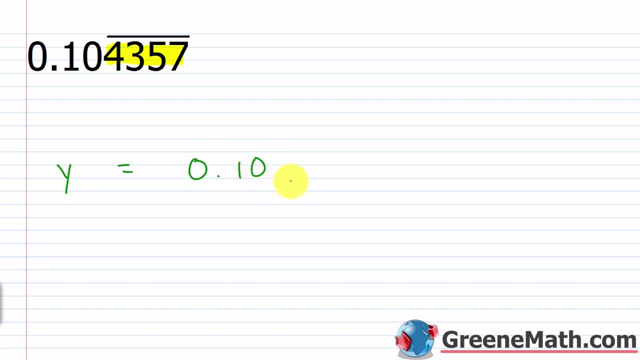 again 0.10.. I'm going to write it in more compact form now that we understand what's going on. So 4357, with the bar over the 4, the 3,, the 5, and the 7.. So I'm going to multiply both sides of this equation. 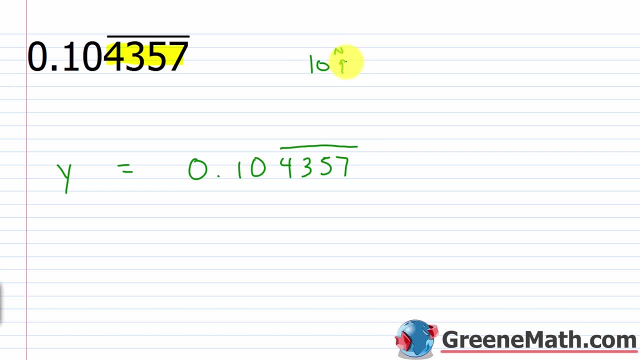 by 10, raised to the power of n Again, where n is the number of digits and the repeating string. So in this particular case we have 1,, 2,, 3,, 4 digits. So I'd multiply by 10 to the power of 4.. So 10 to the power of. 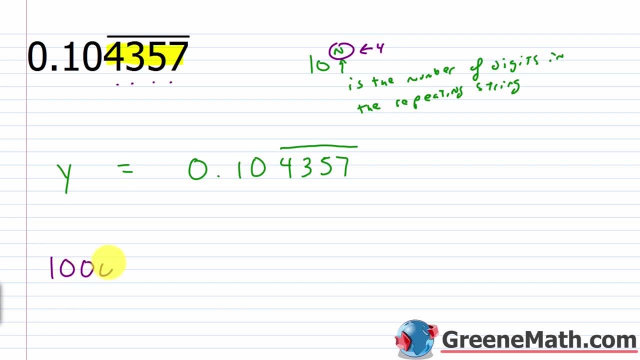 4, which is a 1, followed by 1,, 2,, 3,, 4 zeros. So I'd have. 10,000y is equal to. this would move 1,, 2,, 3,, 4 places to the right. So I would have. 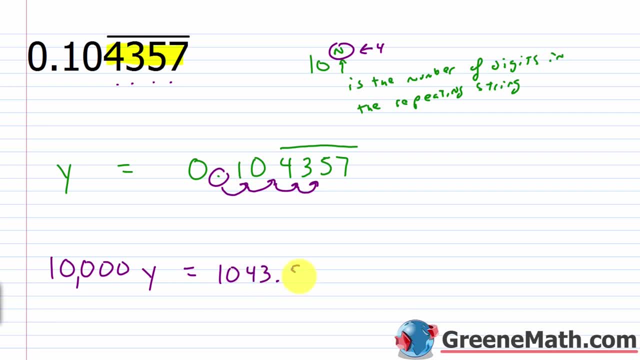 1043.. I'd have 5,, 7 and then what I'd have is the repeating pattern starting. So I would have 4, 3,, 5,, 7.. And I'll put a bar over the 4,, the 3,, the 5, and the 7.. 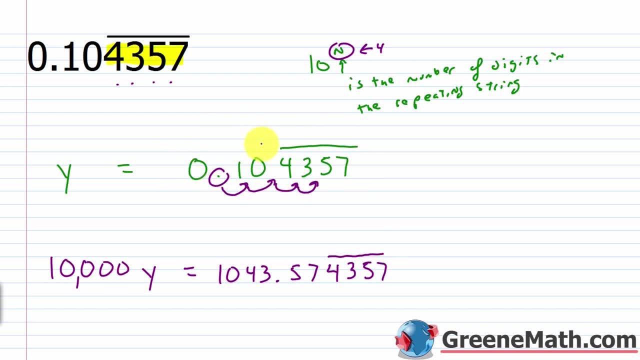 And again, now I want to subtract this value away from each side of the equation. So if I subtract that away over here, I'd have 0.104357, with a bar over the 4,, the 3,, the 5, and the 7.. 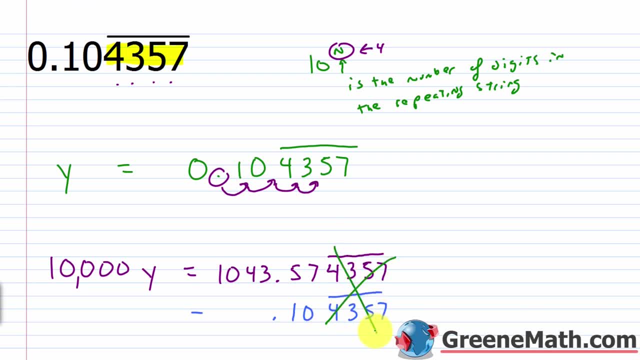 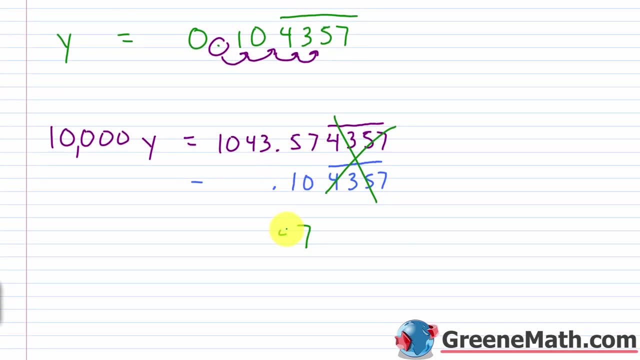 And we know that this part would cancel. Right, That's gone. Let me scroll down a little bit And over here, 7 minus 0 is 7.. 5 minus 1 is 4.. Put my decimal point there. Bring everything else down: 3,, 4,, 0,, 1.. 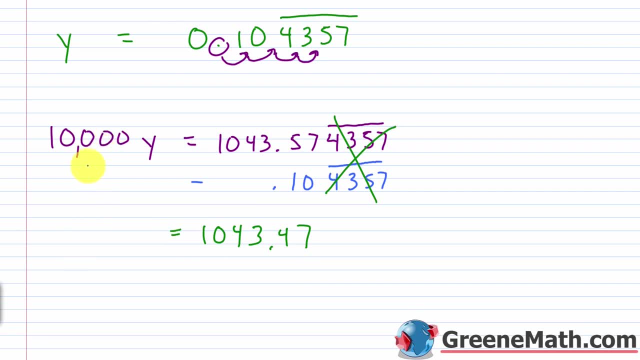 And this would be equal to Over. here I'm going to subtract away y. Remember y equals this. So I'm subtracting away the same thing from each side of the equation. So that's going to give me 9,999y. 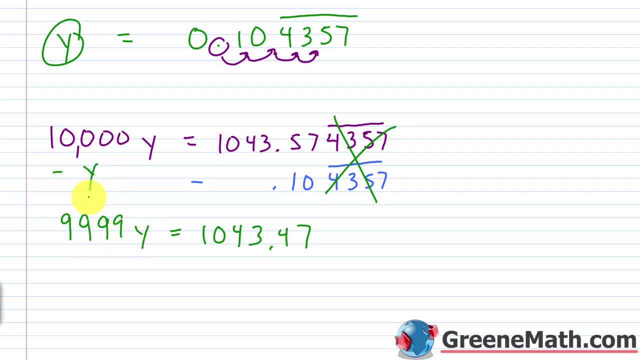 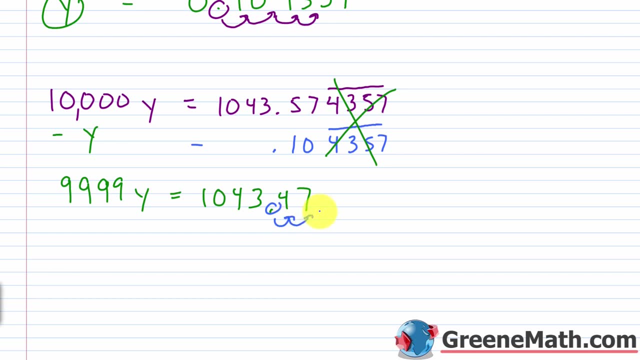 Let me put minus y here. Now, the next thing is I want to just clear this decimal point. So let me multiply by 100 so I can move this 2 places to the right. So that would give me 104,347.. Then on this side, 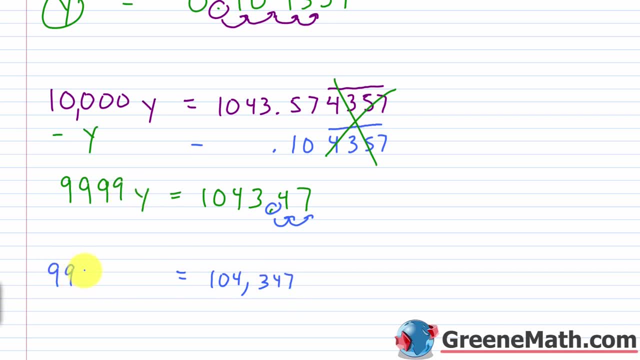 I'm multiplying by 100 as well, So that would give me 999,900y. Then for my final step here, I'm simply going to divide both sides of the equation by 999,900.. And I'll get my final answer here, Which is that y is equal to. 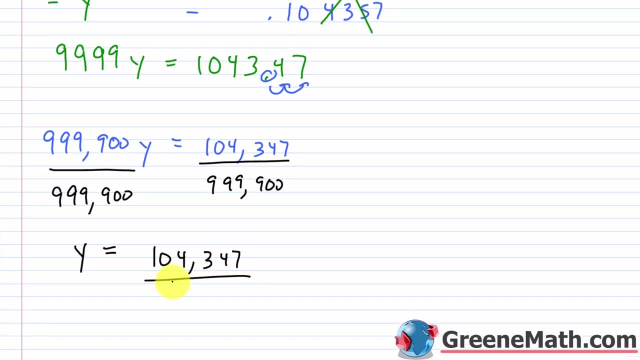 104,347.. over 999,900.. Now, 104,347 is a prime number, So we're not going to be able to do anything to reduce this fraction. So let me just erase some stuff here. So we come back up to the top. 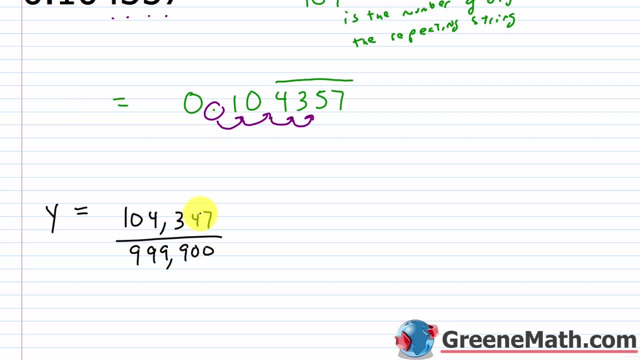 And since y is equal to this, I can replace y with this and put 104,347 over 999,000.. Again, this is equal to what we originally started with. We have 0.10, with the 4357 repeating forever. Let's take a look. 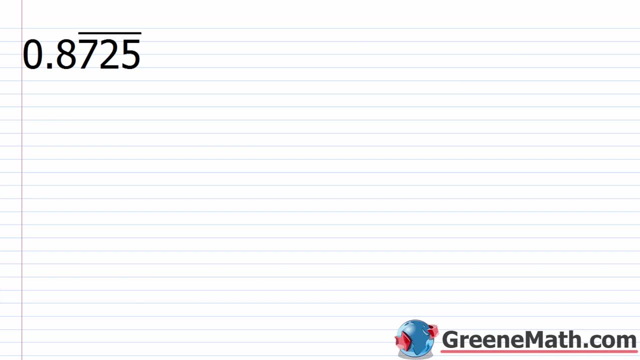 at one final problem here. So we have 0.8725 or 8725.. Those three digits repeat forever. So again, I want to set this equal to a variable. So let's pick x again. So x equals 0.8725. 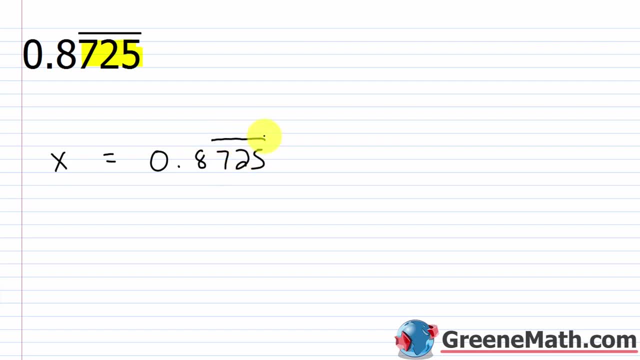 or 8725. Again, where there's a bar over the 7,, the 2, and the 5.. Then let's multiply both sides of the equation by 10, raised to the power of n, Where again n is the number of digits in the repeating string. So in this, 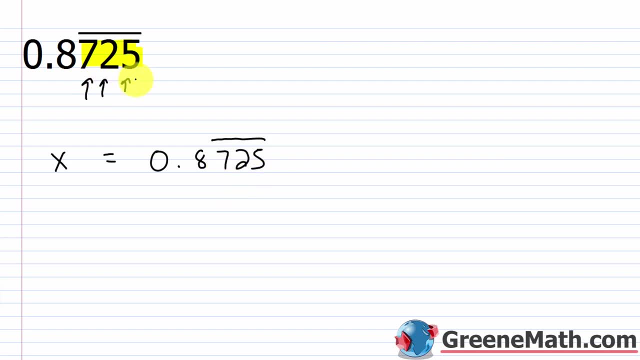 case, that's 3.. I have 1,, 2, 3 digits, So I'd multiply by 10 to the third power or 1000. So I'd have 1000x is equal to. this would move 1,, 2, 3 places to the right. 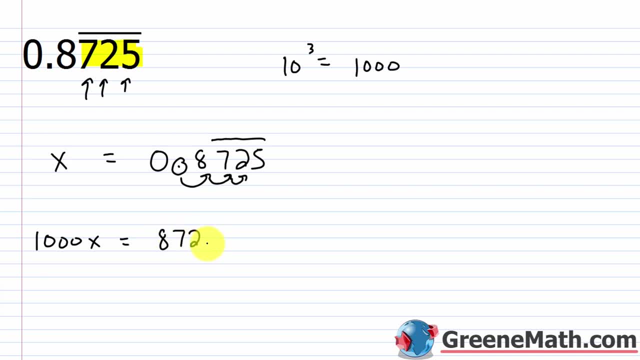 So I would end up with 872.5, and then I would start my 7,, 2,, 5 repeating forever. So let me put the bar over this Now. what I want to do from here, I want to subtract this value from each side of the equation. So over here. 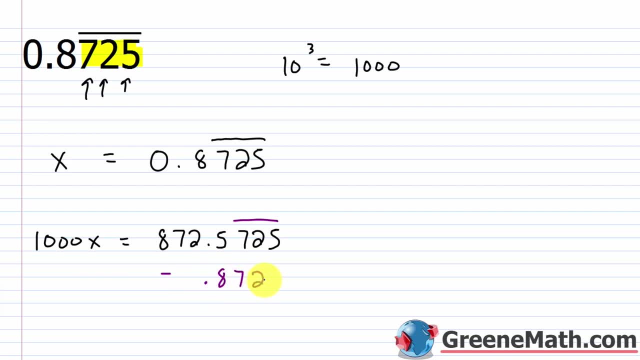 I'm going to subtract away 0.8725, where again there's a bar over the 7,, the 2, and the 5.. And then over here, because x is equal to this, I'm going to subtract away x. I'm subtracting away the same thing from each side of the equation. So on the left I get. 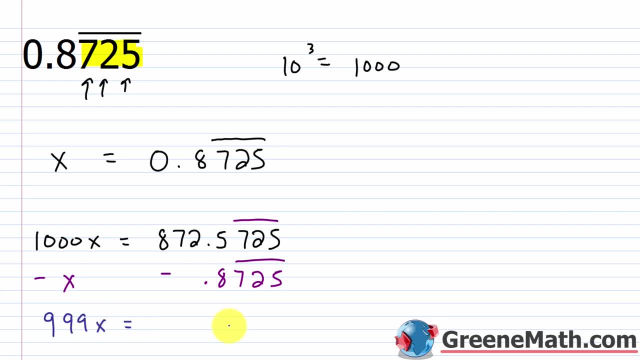 999x On the right. this is going to cancel, and I'll borrow here: 15 minus 8 is 7, and I'll bring down my decimal point, and then I'll bring down a 1,, a 7, and an 8.. So let's. 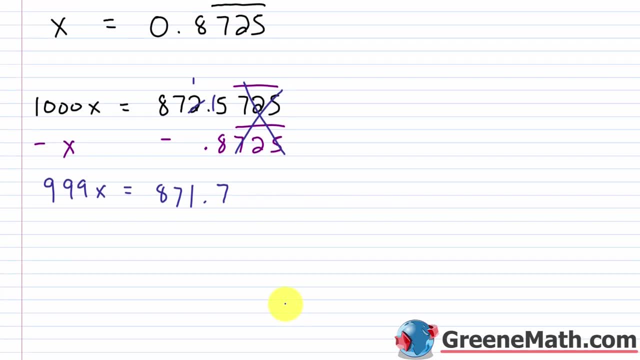 scroll down and get a little room going And I'm going to move this to the right one, which means I'm going to move this to the right one, Just multiplying both sides by 10.. So I'm going to have: 9,990x is equal to 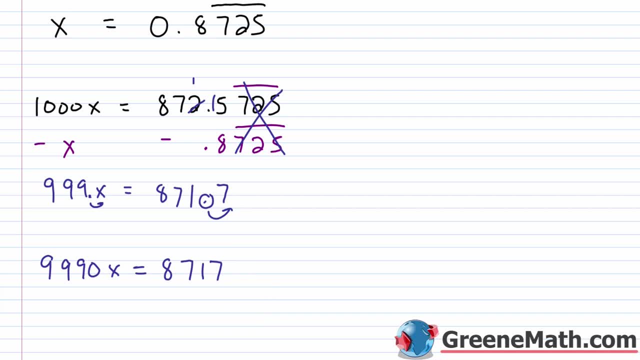 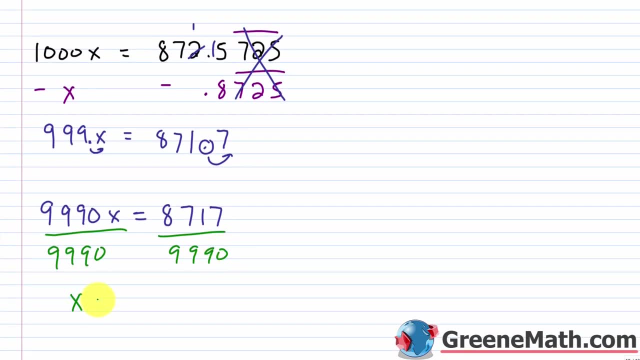 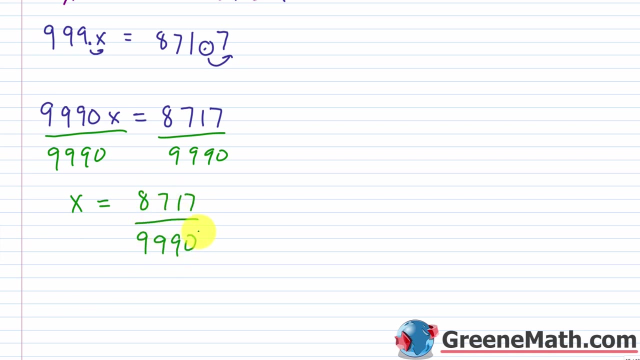 8,717.. Now, as a final step, I'm just going to divide both sides of the equation by 9,990 and I'll get that x is equal to 8,717 over 9,990.. Now, if I factor this number right here, 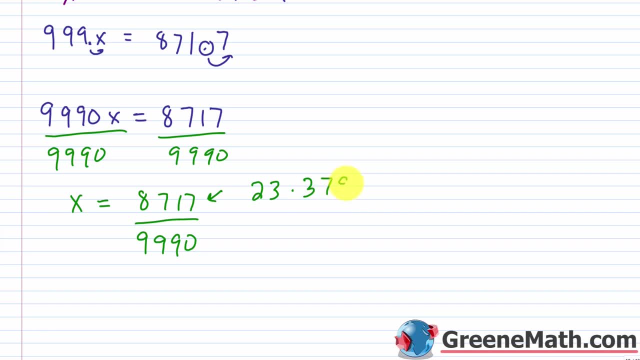 I would get 23 times 379.. And if I factor 9,990, I would get 2 times 3 times 3 times 3 times 5 times 37. So they don't share any common factors other than 1.. So this would be as simple. 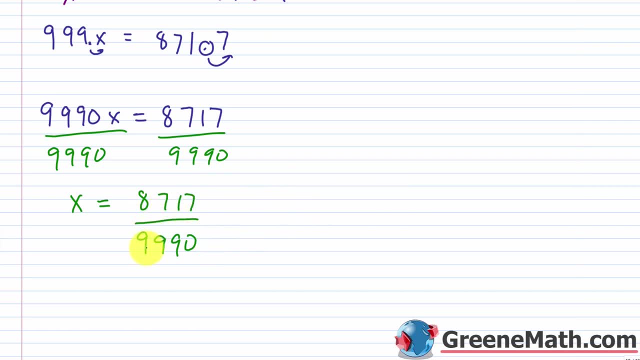 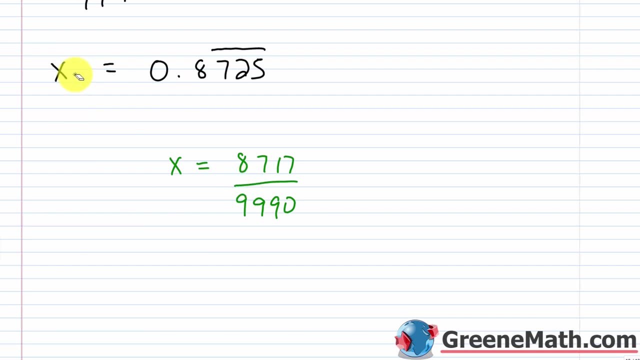 as we can make it, We have 8,717 over 9,990.. And let me just copy this real quick. And again, because x is equal to this, we can say that this value here, 8,717 over 9,990. 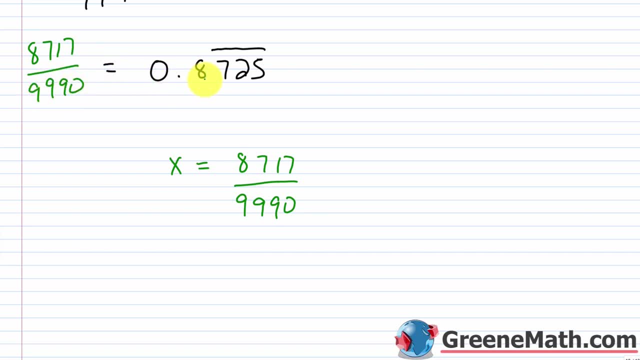 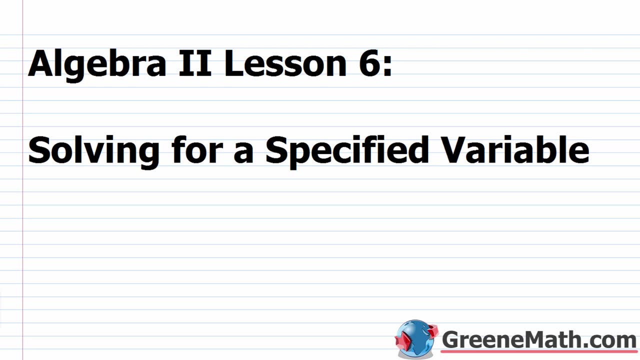 is equal to 0.8725, where the 7,, 2, and 5 repeat: forever and ever and ever. Hello and welcome to Algebra 2, Lesson 6.. In this video, we're going to learn about solving for a specified variable. 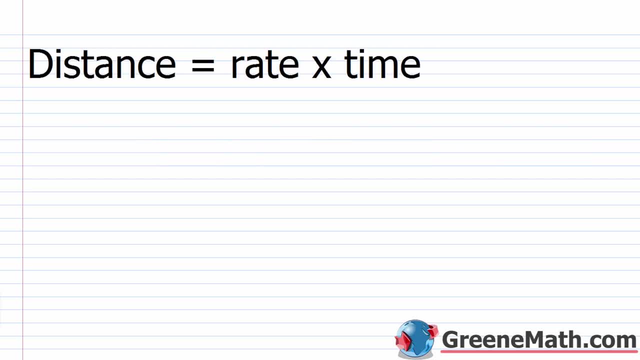 So in many situations we are given equations with no numbers involved. Now in this lesson we're going to talk about some basic formulas where we have equations where the variables describe a relationship. Let's start out by looking at the distance formula, And you'll probably recall this. 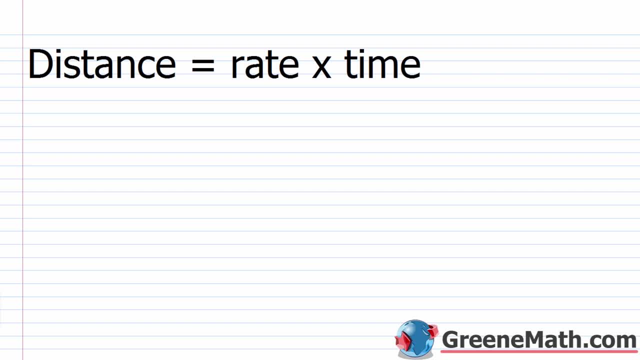 formula from your Algebra 1 course, because we use it on our motion word problems. So we have that distance, which is generally represented with d, is equal to the rate of speed, which we represent with r, times the amount of time traveled, which we represent with t. Now we've all been on a road trip. 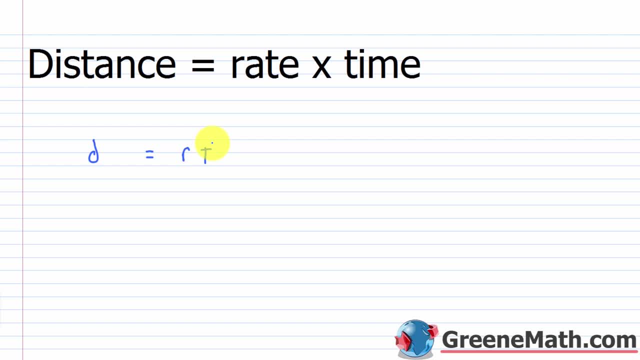 before. and let's say you're on a road trip and you're traveling at 80 miles per hour and you do this for 3 hours. Well, you can plug that into the distance formula and you're going to realize that you went 240 miles. So again, all I would do is I would plug in. 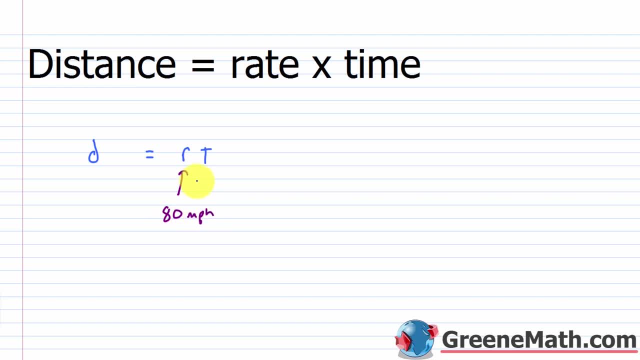 I'm going 80 miles per hour. That's my rate of speed. My time for this trip is 3 hours, So 3 hours Now. forget about the units for a second. just multiply the numbers. If I multiply 80 times 3, I get 240. 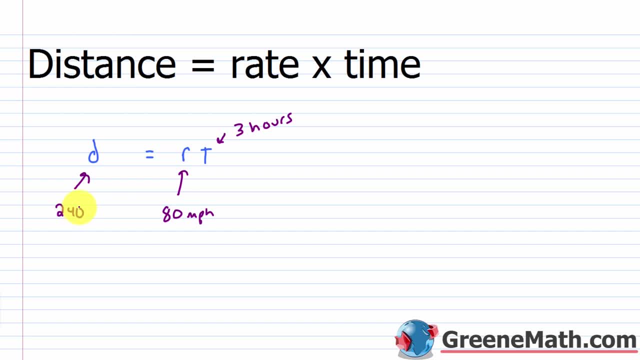 And now you can think about the units. If I'm traveling in miles per hour, then I went 240 miles. That's going to be my distance. So we can see that this distance formula is very, very straight forward. But one thing that we can do: 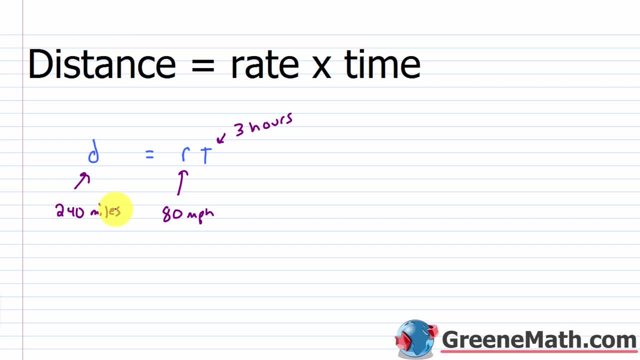 is, we can manipulate this formula and we can solve for the rate of speed or we can solve for the time traveled. So let's say I came up with a different scenario and I had different inputs. Let's say that in this scenario that I gave you a distance, 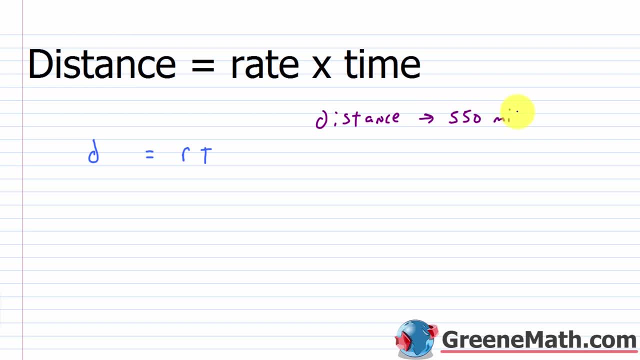 that was 550 miles, So that's how far you traveled And let's say, the amount of time it took to go 550 miles was 11 hours, So your time is 11 hours Now in order to get a solution here for r. 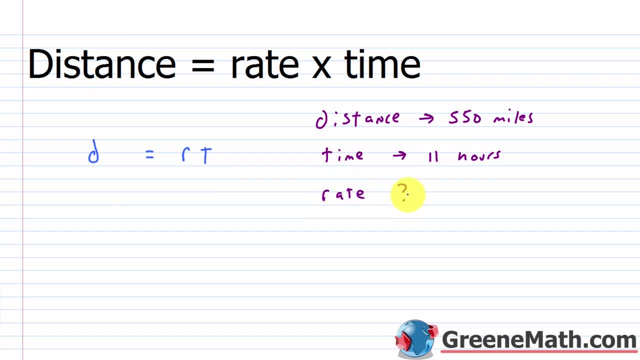 because the rate of speed right now is unknown. what I would want to do is solve this formula for r. So what I'm going to think about here is just treating t as if it's the coefficient of r. If I saw something like, let's say: 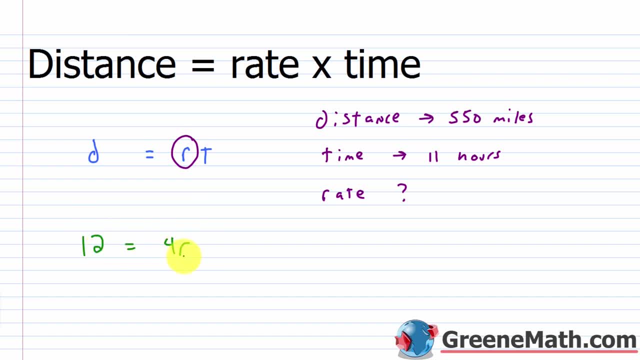 12 is equal to 4r. If I want to isolate r, we know we divide both sides of the equation by 4 and we get 3 is equal to r. Well, it's no different here. If I want to isolate r, all I'm going to do is divide both sides of the equation by t. 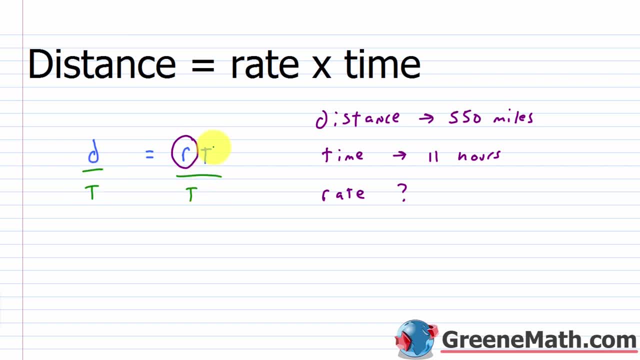 It doesn't matter that it's a variable in this case. So this will cancel with this and I'm going to have that r or the rate of speed is equal to the distance over the amount of time traveled. So now that I have it solved for r, what I 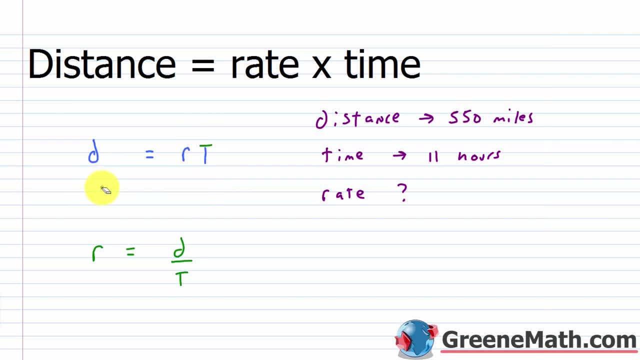 can do. let me just kind of rewrite this. what I can do is I can plug in my inputs. I can plug in 550 miles here and I can plug in 11 hours here, And if I think about the numbers there, 550 divided by 11 is going to give us 50. 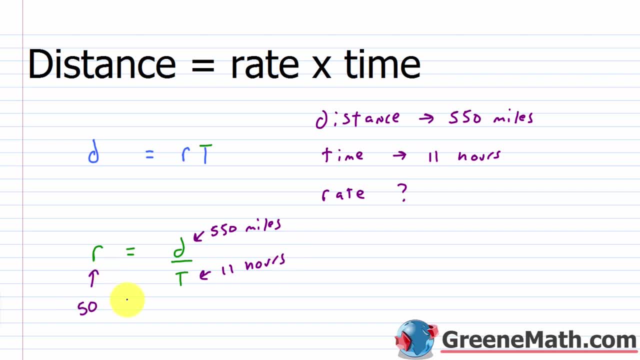 So I know my r there is 50 and when we think about the rate in terms of the units, we're talking about miles per hour. So miles per hour. We have miles here, we have hours here, so that's going to be miles per hour. So my rate is 50 miles. 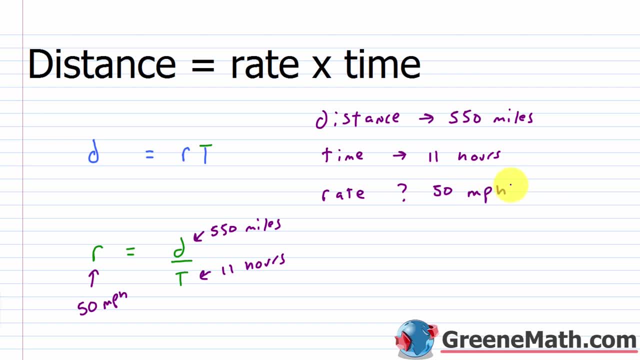 per hour. Now let's say I gave you another scenario- Let's erase this real quick- And let's say that I now gave you a distance. Let's say it's 300 miles. And let's say I gave you a rate. Let's say the rate is 60 miles per hour. 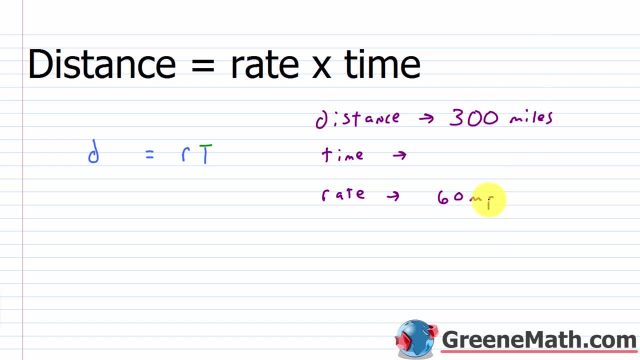 And I asked you for a time. So now this guy is the unknown, So I can solve the formula for time. So if I want to solve for time, I just divide both sides of the equation by r And I'm going to get that time. 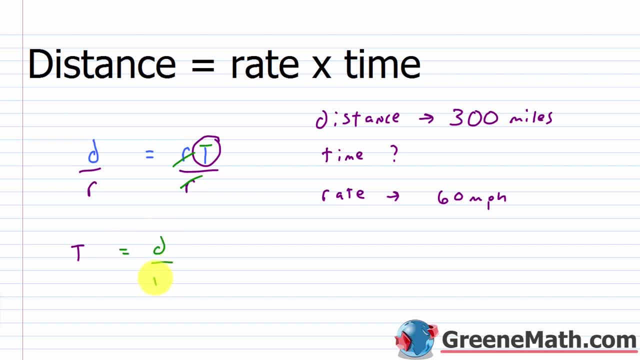 is going to be equal to distance over rate. So once I have that I plug in. So I'm going to plug in for distance, that's 300 miles. I'm going to plug in for the rate of speed, that's 60 miles per hour, And so 300 divided by. 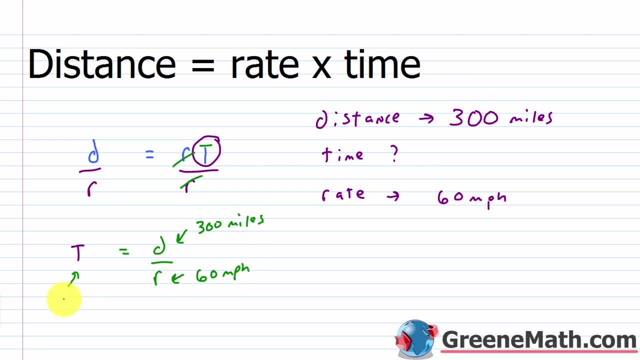 60 is going to give me 5.. So t or time is 5, and again we have miles and we have miles per hour. so we're talking about 5 hours here. So the time is going to be 5 hours. So that's just one example of how you have. 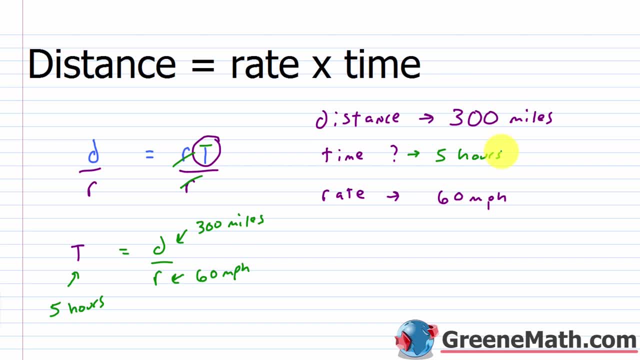 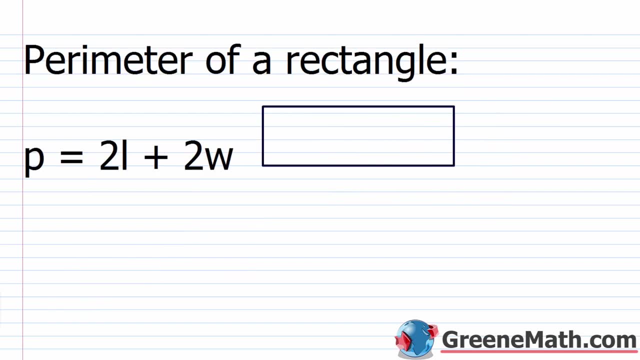 an algebraic formula and you can manipulate it for what you need based on the problem that you're given. Alright, so let's think about another common formula. This is the perimeter of a rectangle, So this is more used in geometry. I know, by the time, 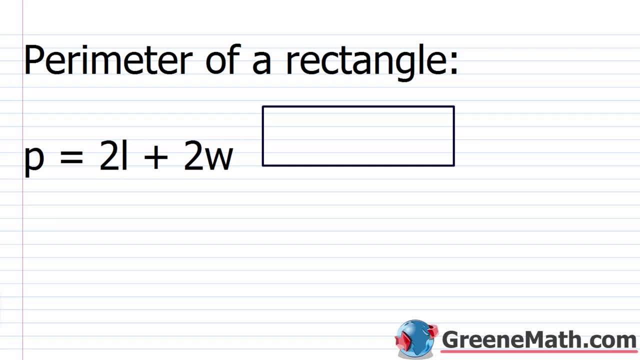 you get to algebra 2? you've taken a geometry course? Maybe you haven't, but the perimeter of a rectangle is given as p, which stands for perimeter, Which is equal to 2 times the length plus 2 times the width. So, as an example, let's say: and this is your width here. 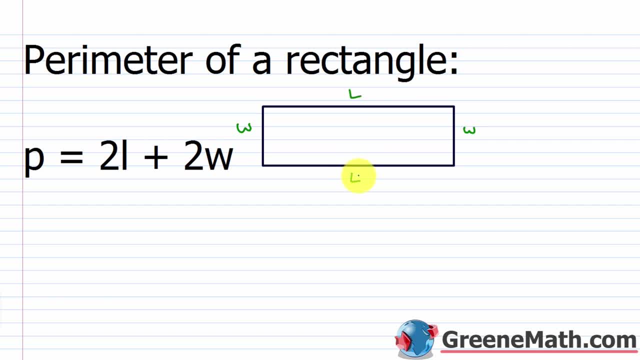 and here. This is your length here and here. Let's say you have a length that is equal to, let's say, 8 feet, And let's say you have a width that is equal to, let's say, 4 feet. If I told you to calculate the perimeter, you just need some basic arithmetic. 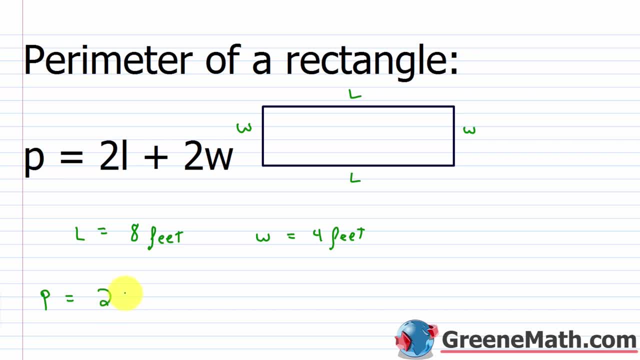 You're going to plug in. So the perimeter is going to be equal to 2 times my length is 8 feet, So I'm just going to put an 8 in. I'll deal with the units in a minute. Plus 2 times my width, I have 4 feet. 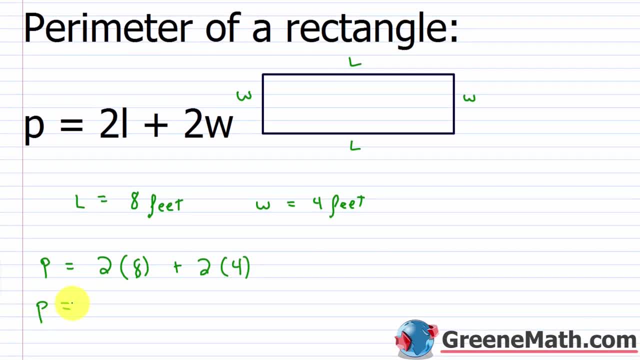 So I'm going to put 4 in. So my perimeter of p is equal to 2 times 8, which is 16, plus 2 times 4, which is 8.. 16 plus 8, we all know, is 24.. So the 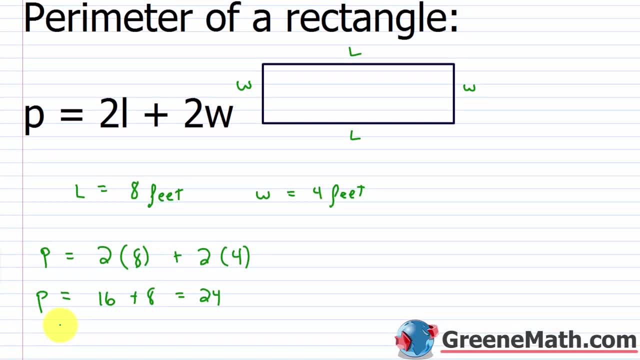 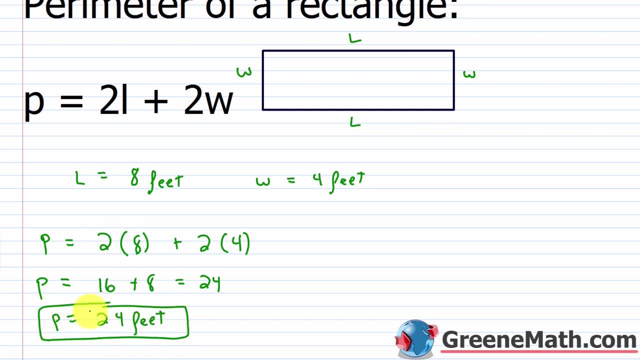 perimeter in this case, if we think about the units as well, would be 24 feet. Ok, 24 feet, Now that's easy to calculate. but what if I gave you a different scenario? Let me erase this real quick, And let's say that I gave you a scenario where I told you what the 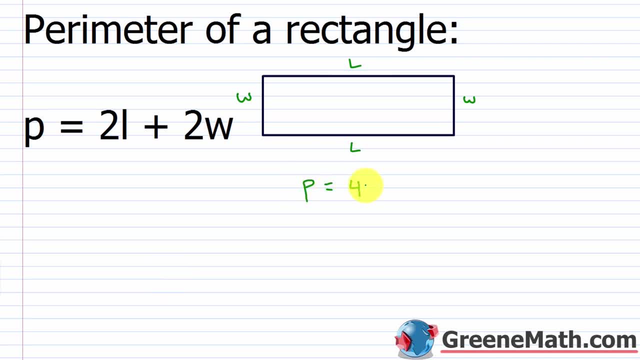 perimeter was. Let's say, the perimeter is now 40 feet And let's say I gave you one of these. Let's say I gave you the width and I said that the width is going to be 7 feet. Well, how would I find out what the length is? So my l 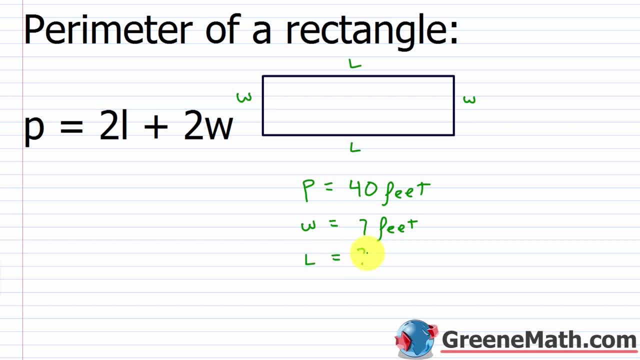 here is unknown. Well, I can solve the formula for length. And how do I do that? Well, I want to get this term by itself to start. So that means I would subtract 2w away from each side of the equation. This would cancel, And on the left I would have. 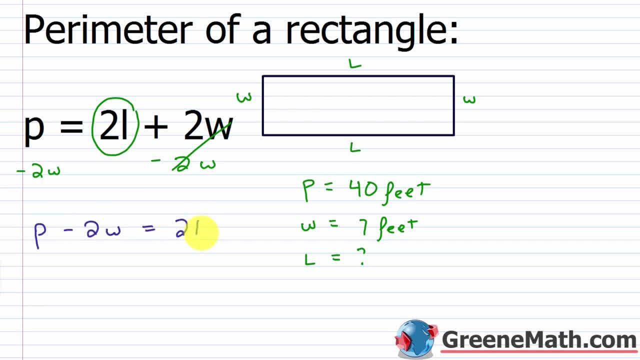 p minus 2w is equal to 2l. Now, to get l by itself, I have a coefficient, I have that 2 there, And so I'm going to do the same thing I've been doing. I'm just going to divide both sides. 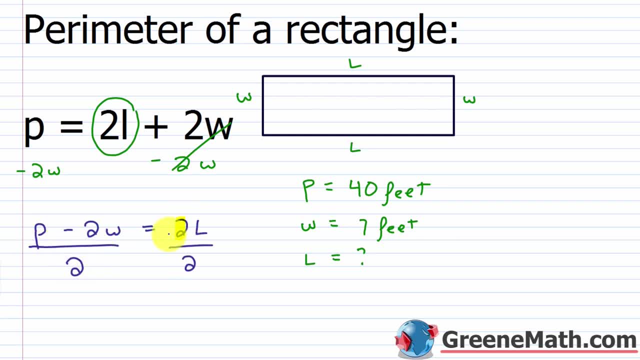 of the equation by 2. So that l can be by itself. So this will cancel with this And I'll have l is equal to. I'll have p, or perimeter minus 2 times w, or width over 2.. Now all I need to do, once I've solved for length, is just: 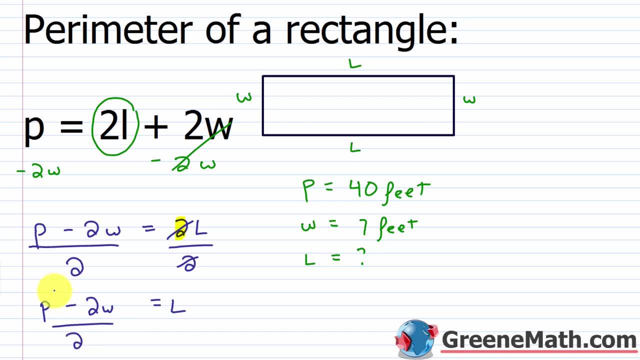 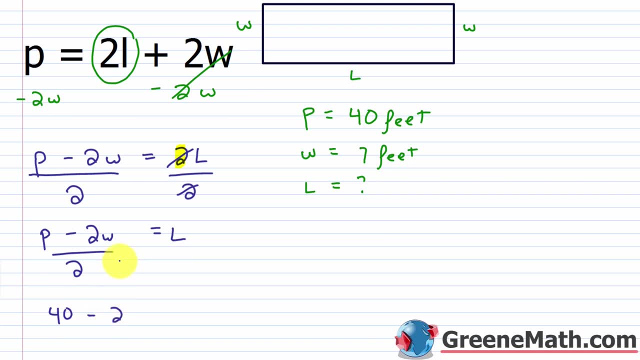 plug in. So I know the perimeter is 40 feet, So let me scroll down and get a little room going. So for p I'm going to plug in a 40 and I'll deal with the units in a minute Minus 2 times. for the width I'm going to plug in. 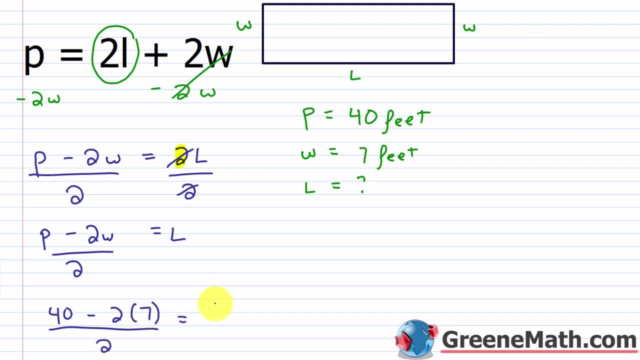 a 7. And this is over 2. And this should give me my length. So 2 times 7 is 14.. So let's just erase this and put 14.. 40 minus 14 is 26.. So I'd have 26. 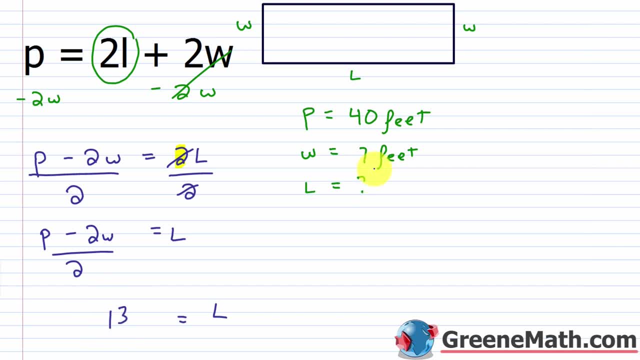 over 2, which is 13.. So my length here is 13.. And again, you want to use the units. so it would be actually 13 feet Right, 13 feet. Now you can check that with the original formula. Let me kind of erase everything here, And if I go to the original formula, 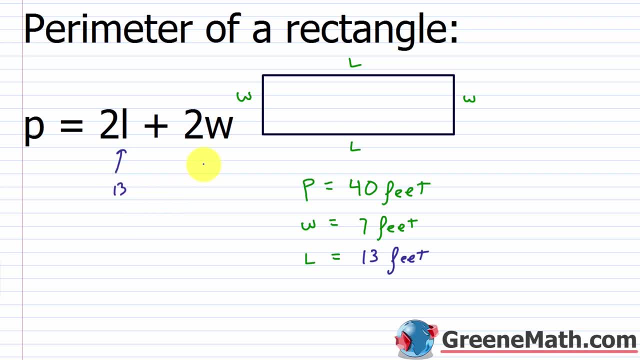 if I plugged in a 13 here and I plugged in a 7 here, Would I get a perimeter of 40?? And again, we're dealing with feet in terms of the units. So 2 times 13 is 26, plus 2 times 7, which is 14.. Yeah, that would work out. 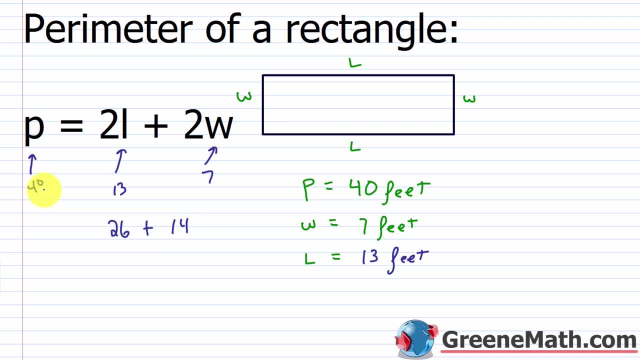 26 feet plus 14 feet would in fact give me 40 feet. So that works out. Now, as another example, what if I am given the perimeter and I'm given the length? Well, now I need to solve for the width. So let's say: 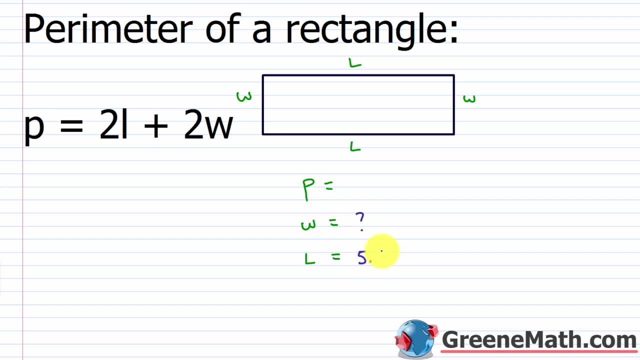 this is unknown. Let's say, I give you a length that is 5.5 feet And I give you a perimeter that is 16 feet. Well, now I want to solve the equation for W or the width, And it's the same thing, it's just. 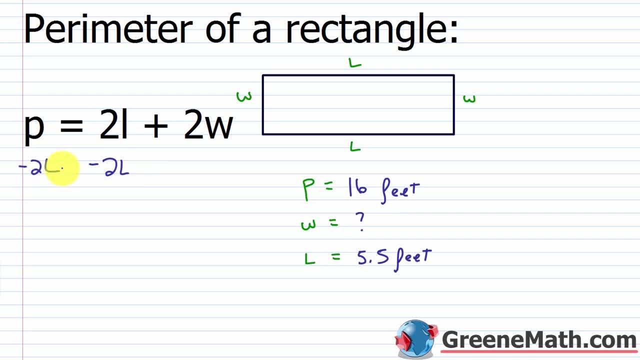 a little bit different. I'm going to subtract away 2L from each side of the equation, So that's going to cancel. I'll have P, or the perimeter minus 2 times L, or the length is equal to 2 times W, or 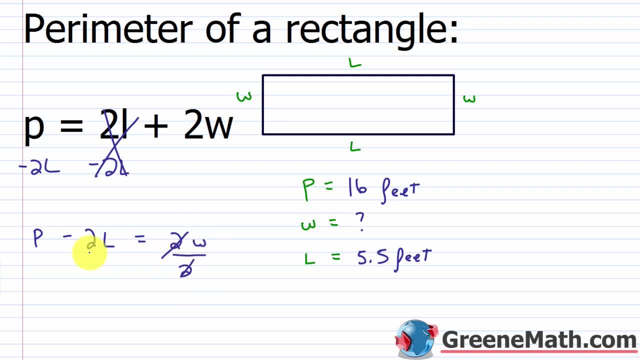 the width And again divide both sides of the equation by 2, so you can isolate W And what I'm going to have is that W, or the width, is equal to perimeter minus 2 times the length over 2.. So if I just plug in my inputs here, If I plug in a 16 here, 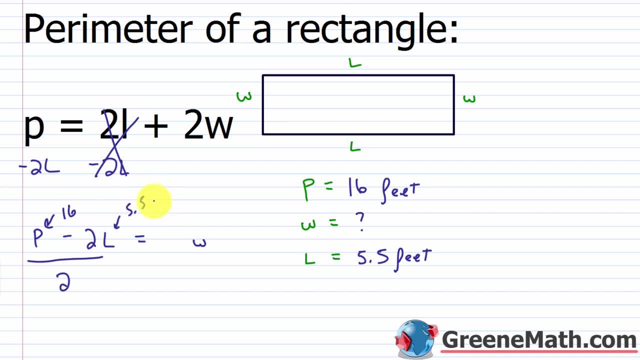 and I plug in a 5.5 here. What's that going to give me? Well, I would have 16 minus 2 times 5.5 is 11.. So this would be 11.. So you'd have 16 minus 11, which is 5.. 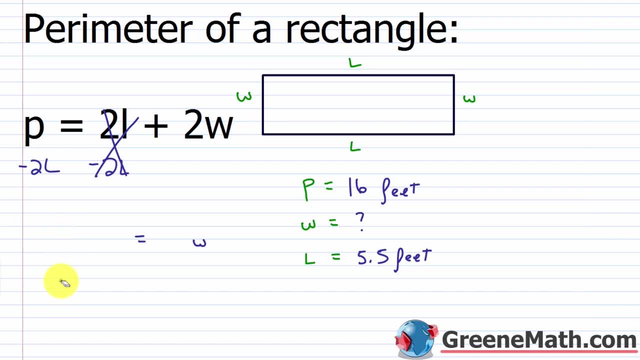 So you'd have 5 halves or 2.5 as a decimal, And don't forget the units. so this would be 2.5 feet. So my width is 2.5 feet. Let me erase this And we'll put 2.5 feet. 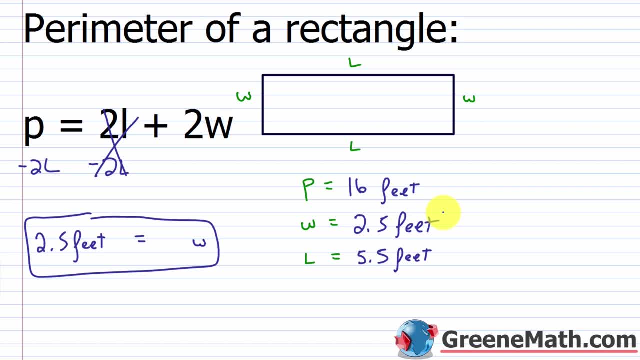 So again, another great example of how we have an algebraic formula. We have more than one variable that's involved And we can solve for whatever variable that we want. It's just based on the information that's given in the problem and what we need to find. Alright, so here's. 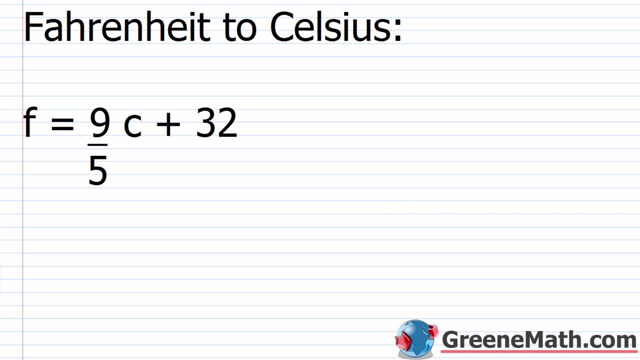 another great example: We have Fahrenheit to Celsius. So if you live in America, like I do, all of the temperature readings that you get are generally going to be in Fahrenheit. I know if you take a science class you get a lot of stuff in Celsius and things like that. but 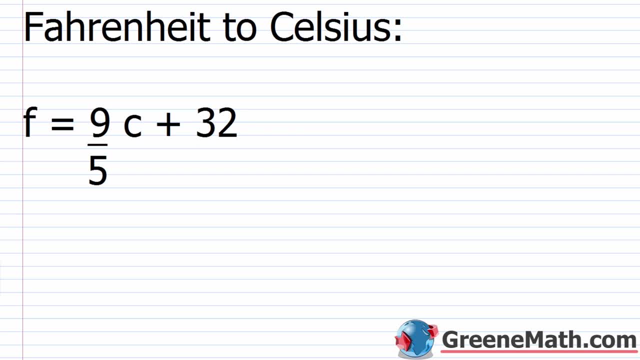 in general, when we report a temperature here in America, we get Fahrenheit. Now, if you're in another part of the world, you might get it in Celsius, So you need to be able to convert back and forth. So this is the formula: If I give you a temperature in Celsius, you plug it in. 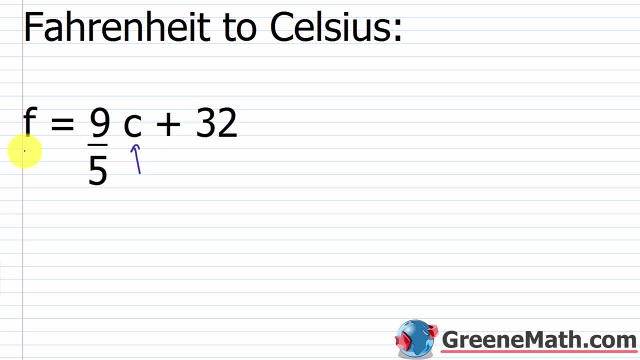 you multiply it by 9 fifths, you add 32, you get a temperature in Fahrenheit. So we can try this out. Let's say I wanted to convert 25 degrees Celsius to Fahrenheit And I'm not going to write that, I'm just going to put it to F. So what would I do? 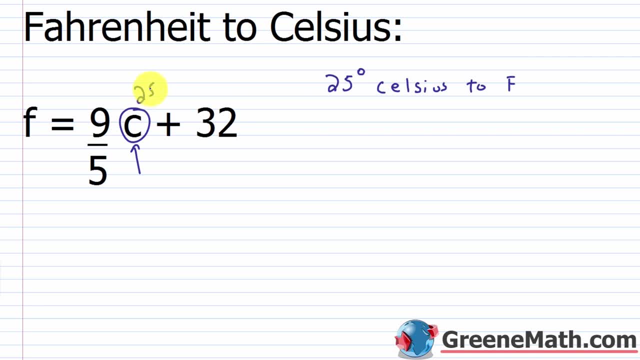 I'd plug in a 25 here. Plug in a 25 here. So my Fahrenheit is going to be equal to. we'd have 9 fifths times 25 plus 32.. We know that this would cancel with this and give me 5.. 5 times 9 is 45.. 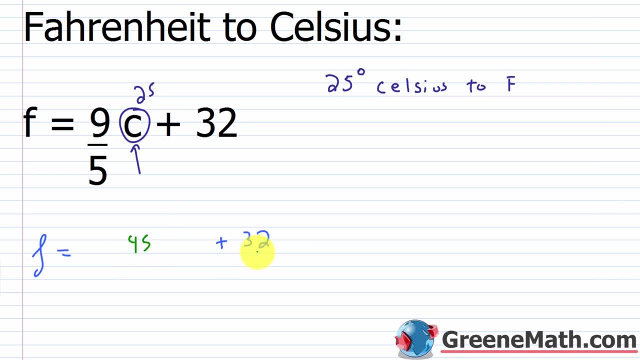 So you're looking at 45 plus 32. And we can do that in our head. 5 plus 2 is 7.. 4 plus 3 is 7. So 25 degrees Celsius would be 77 degrees Fahrenheit. So those. 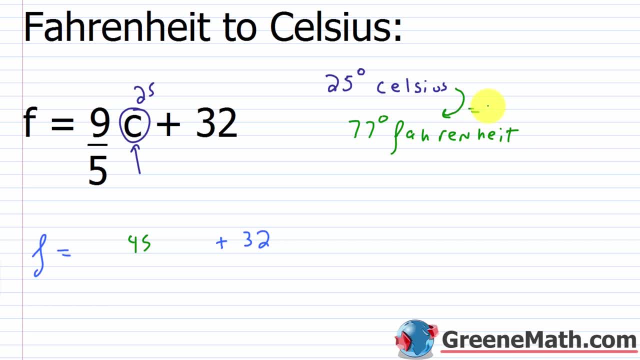 two are equal to each other. Now, let's say that I gave you a temperature in Fahrenheit and I wanted to go to Celsius. Well, I would need to solve the formula for C. So how would I do that? Well, I want to isolate C. Now F is isolated. 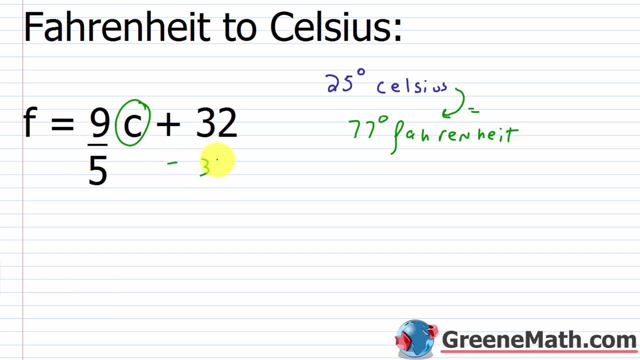 So let's start out by just isolating this, and we'll subtract 32 away from each side and do that, So I'll have F minus 32 is equal to 9 fifths C, And what I want to do here is I have a 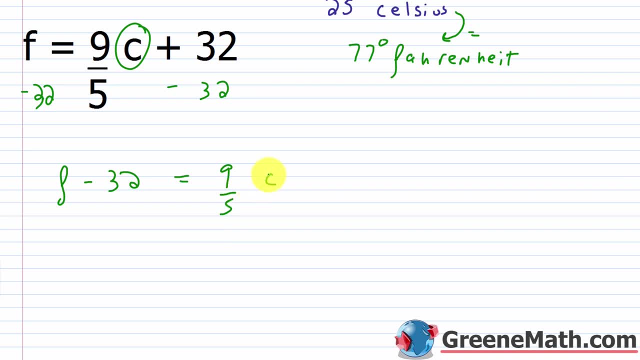 fraction as the coefficient for C. So when I have a fraction I can just multiply by the reciprocal. So I can multiply by 5 ninths. And of course what I do to one side I've got to do to the other. But this is going to cancel itself out. This is going to be 1.. 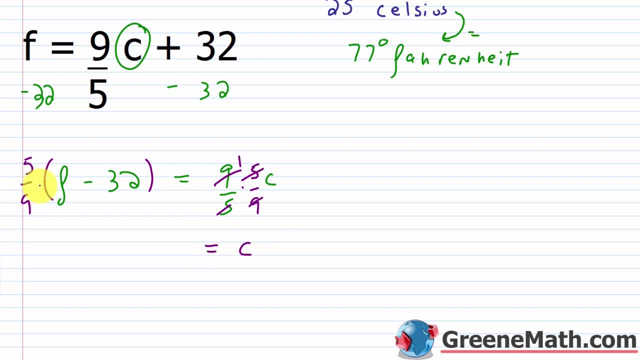 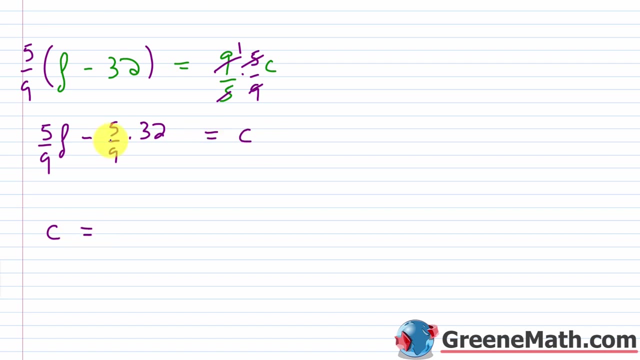 So on the right side I have C. On the left side I'd have 5 ninths times F minus 5 ninths times 32.. Now of course, I can write this more cleanly by saying that I have C is equal to. I just switch what side it's on. I like my variable to be on the left. 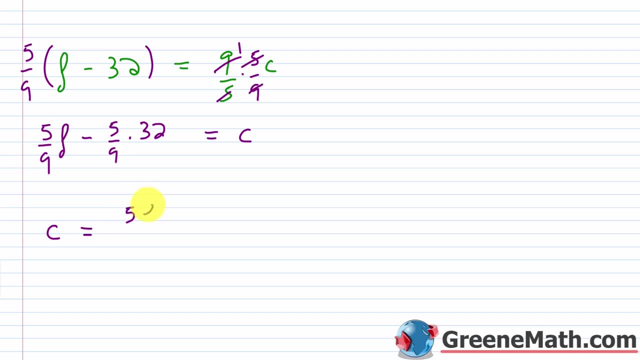 Over here. I would have 5 F minus 5 times 32 is 160.. So 160.. And this is over the common denominator of 9.. Now I just showed you that 25 degrees Celsius was 77 degrees Fahrenheit. Let's try it out in this formula. So let's plug in a 77 here. 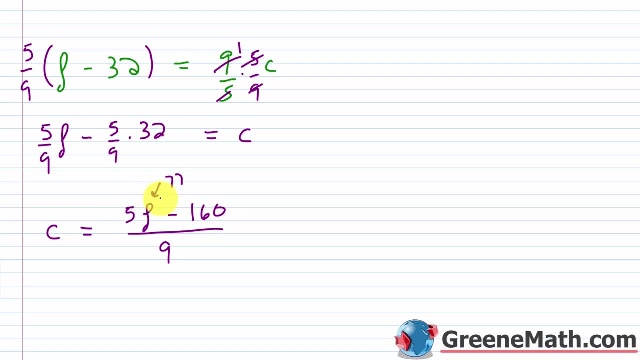 And see if we get 25.. So 5 times 77 is 385.. So what I'd have is C, or Celsius, is equal to 385 minus 160 over 9.. If I subtract 385 minus 160, I get 225.. So I'd get 225 over 9.. 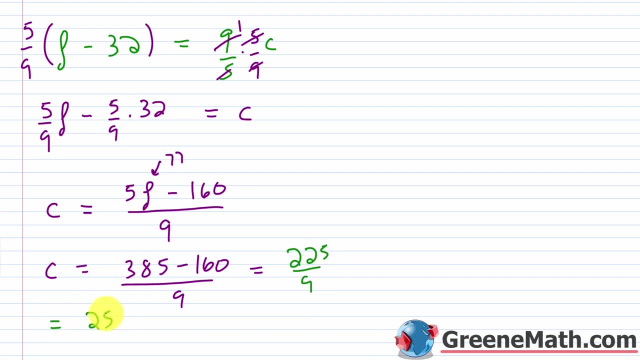 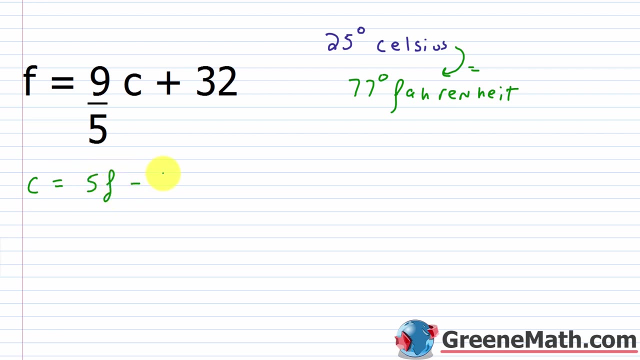 And we know this is going to be equal to 25.. So again, when I go from 77 degrees Fahrenheit back to Celsius, I get 25 degrees Celsius. So let me rewrite this formula: C or Celsius is equal to 5 F minus 160 over 9.. 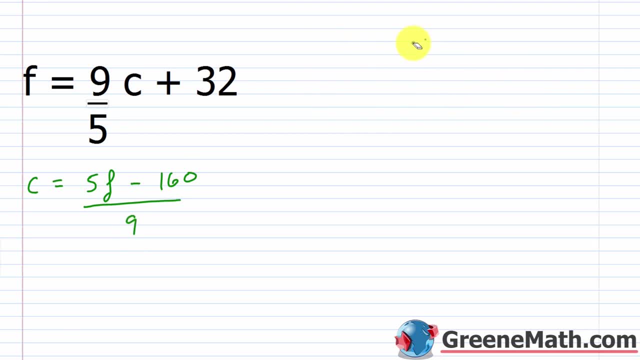 Now let's try just one more. We'll go back and forth. Let's say that I have 37 degrees Celsius And I want to convert this to Fahrenheit. So how many degrees in Fahrenheit? This is actually a very popular temperature that deals with the human body. So if I'm going from Celsius to 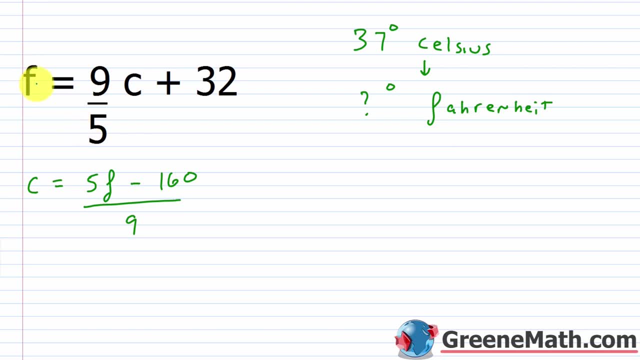 Fahrenheit. I want to plug into this formula here because it's solved for Fahrenheit, So what I can do is I can plug in my 37 here And I would have 37 times 9. fifths, Well, 37 times 9 is 333.. 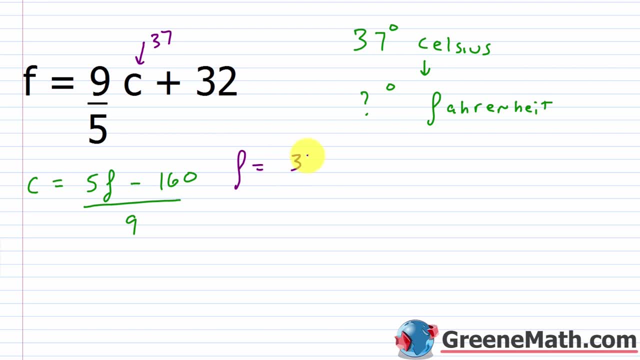 So what this would give me is: F is equal to 333 over 5, plus you have 32 there Now to get a common denominator. I know, if I multiply 32 times 5, I get 160.. So this would be 160 over 5.. 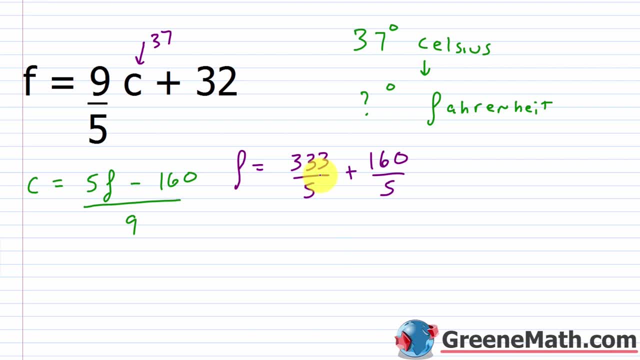 And so 333 plus 160 is 493.. So this would end up being 493 over 5.. But in decimal form you'd end up with 98.6.. 98.6.. So 37 degrees Celsius is 98.6. 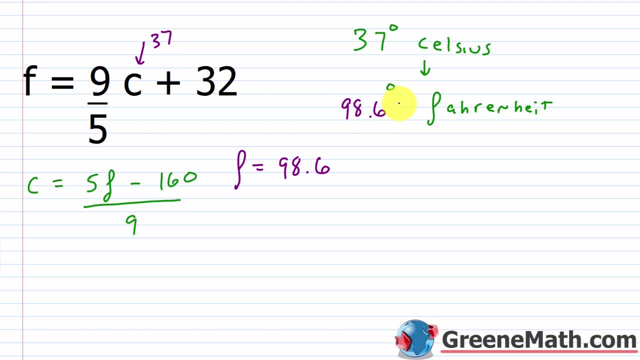 degrees Fahrenheit. Now. this temperature is significant because for most people a body temperature of 98.6 degrees is normal. If I take a thermometer, put it in my mouth, under my tongue, I'm looking for something around 98.6 degrees. So let's just do one more here And all I'm going to do is just convert. 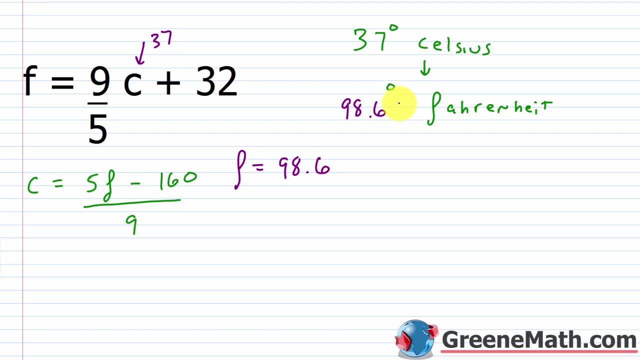 98.6 degrees back to show you that this formula does indeed work. So let me erase this And I'm going to plug in 98.6 here, And 98.6 times 5 is 493.. So 493 minus. 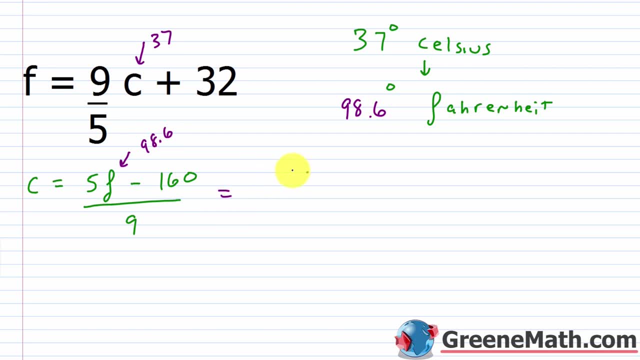 160 would be 333.. So this would be 333 over 9, which we know is 37. So again convert this back and forth. you see that again, 37 degrees Celsius is 98.6 degrees Fahrenheit. So you can see how solving this for Fahrenheit with F. 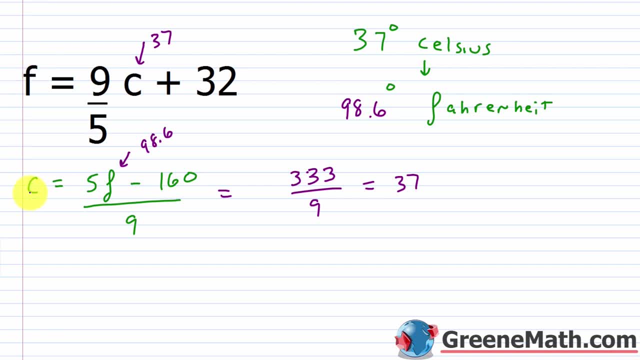 and then solving it for Celsius allows you to attack any problem they throw at you. If they give you a temperature in Celsius and ask for Fahrenheit, you use this one. If they give you a temperature in Fahrenheit and ask for Celsius, you use this one. So it's an ability to go back and forth. 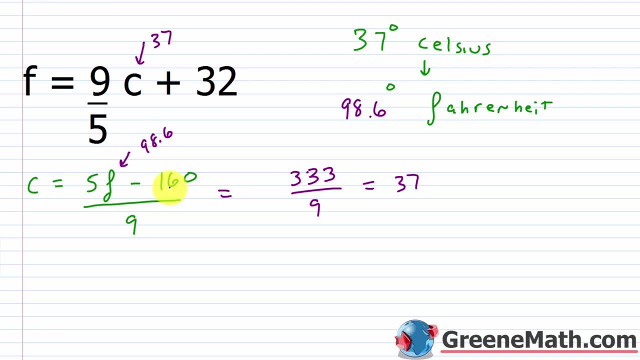 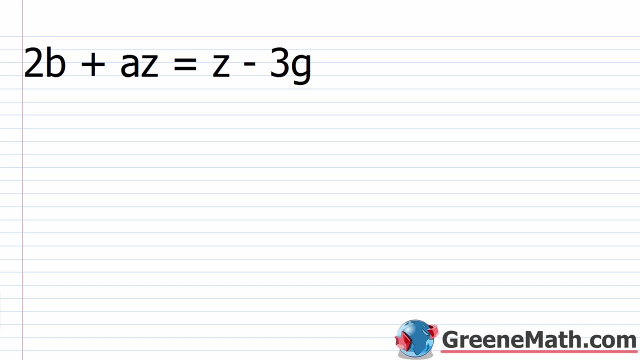 And again, it's just based on the information given to you in the problem as far as what you want to solve for. Alright, for the last problem, let's look at one that's not a generic formula. Let's just look at something you might see on your SATs. 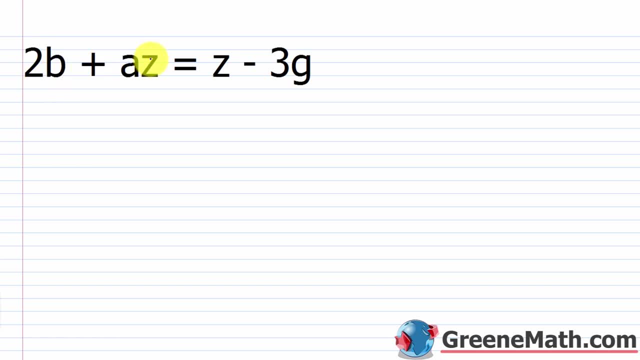 So you might get something that's like this: 2B plus AZ equals Z minus 3G. You might say: what is this? They might say: I want you to solve this for Z, I want you to solve this for B, I want you to solve this for G, So on and so forth. Let's just 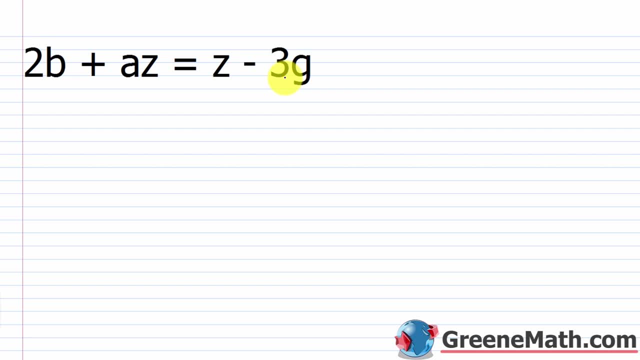 do one and let's just say we're going to solve it for Z, So let's solve for Z. So how do we do that? Well, I've got to isolate Z on one side of the equation. That means I'm going to isolate all the terms with Z in it on. 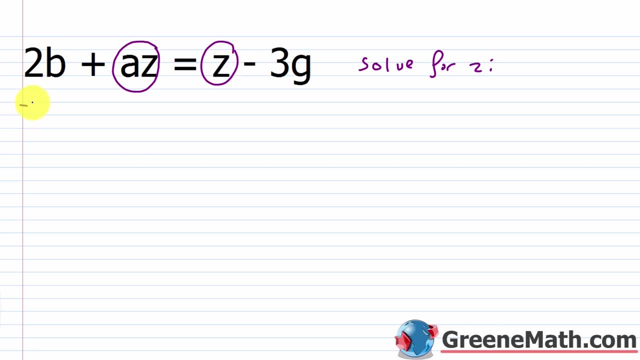 one side, Get everything else on the other. So I can subtract 2B away from each side of the equation And I can subtract Z away from each side of the equation. So this is going to cancel. This is going to cancel. 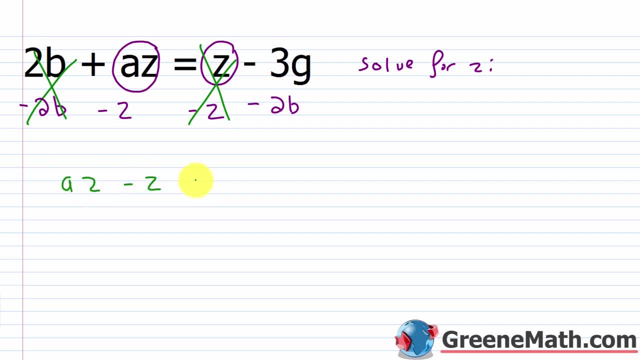 And I will have: AZ minus Z is equal to negative 2B minus 3G. Now how do I get Z by itself? This is tricky if you don't have any experience in Algebra 1. If you've just gotten into Algebra, you might. 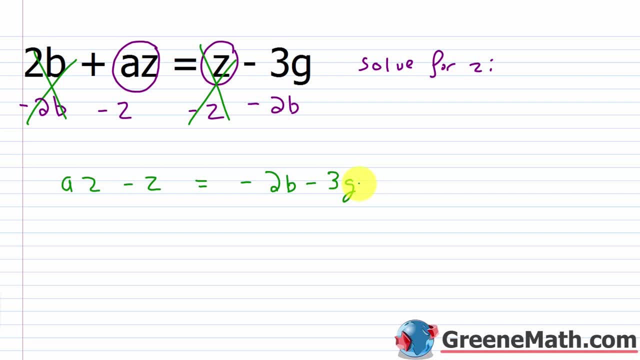 go. what in the world are we going to do? Well, for most of you that took Algebra 1, you know how to factor. If you didn't take Algebra 1, let me just kind of explain briefly what we're doing here. I am able to pull something that's common. 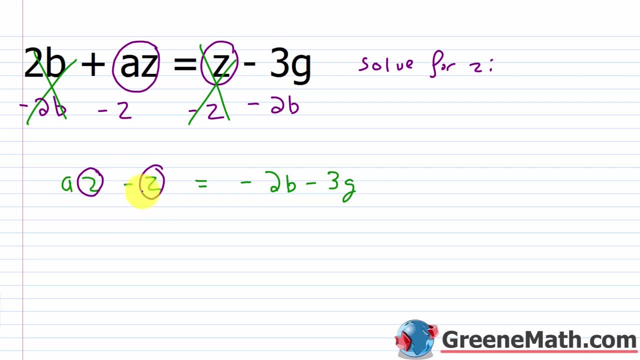 outside of a set of parentheses. So if Z is common to each term here, I can place it outside of a set of parentheses. When I do that, what's going to be left in the parentheses is what was multiplying Z. So here A is multiplying Z, so it's there. Then minus Here you might. 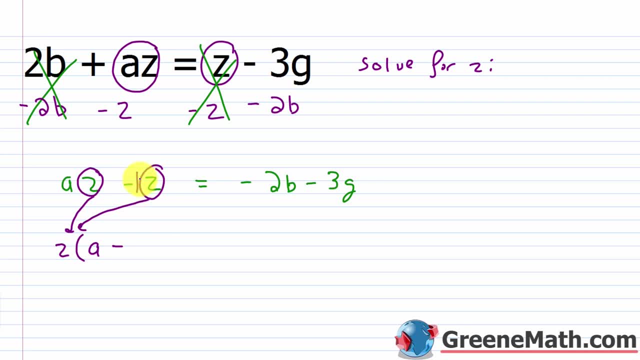 say: well, nothing is multiplying Z. Well, yeah, you always have a phantom 1 there. So really, if I factor out a Z, I end up with a quantity A minus 1.. And you can check that through multiplication Z times A is AZ. 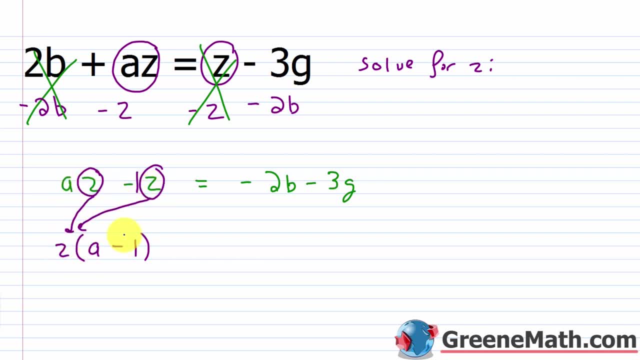 Then minus Z times 1 is Z, So you're back to what you got. So I just wrote this in a different form And another way. you can kind of think about this. Let me kind of erase this real quick. If I had, 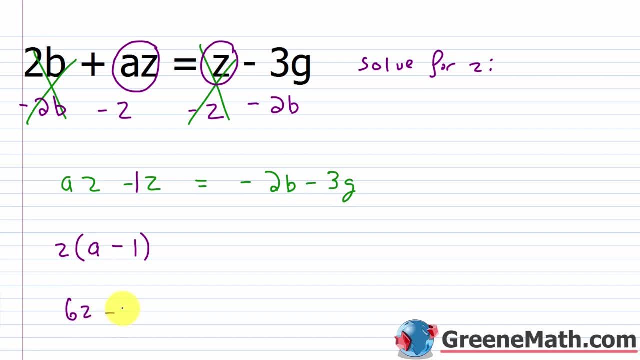 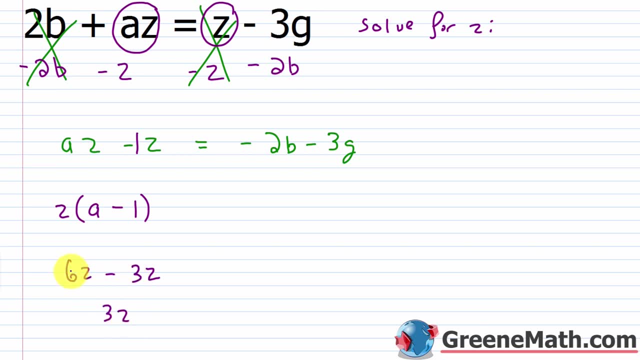 like terms. Let's say I had 6Z minus 3Z. Okay, for example, Here, 6Z minus 3Z would be 3Z, Because I subtracted this minus this: 6 minus 3.. In this particular, 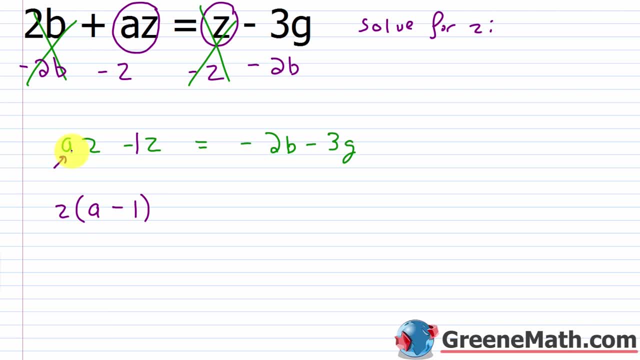 case. I don't know what A is, But if A was 5, for example, I'd have 5Z minus 1Z, That would be 4Z. So if A was 5.. 5 minus 1 would be 4. I'd have a coefficient out there, But I don't have the luxury of that. 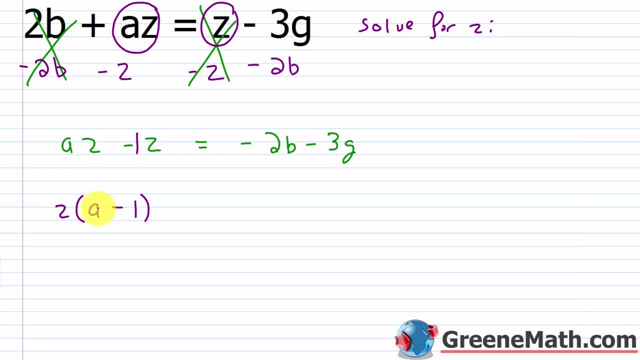 because in this particular case I'm just given A And I don't know what that is. So this is the best we can do: We factor out the Z And we leave it in this form And we say it's equal to negative 2B minus 3G. You might say: 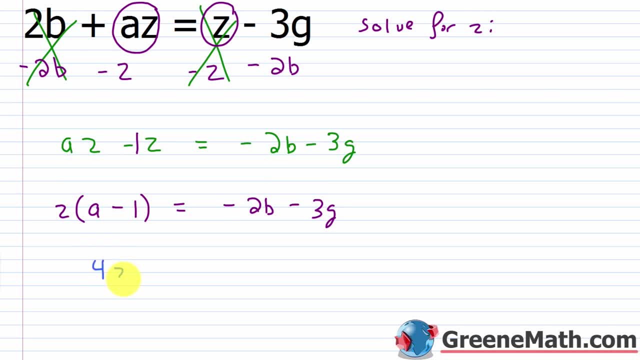 well, how do I get Z by itself? Well, just like if I had, 4Z is equal to something. I divide both sides by 4.. Well, I'm going to do the same thing here. I'm just going to divide both sides by this quantity. 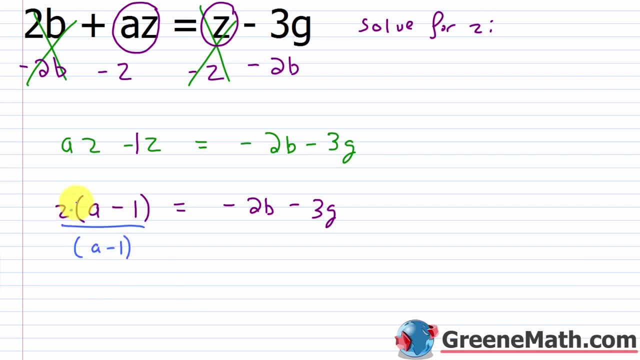 A minus 1.. That is what's multiplying Z. So that's what I'm going to do: I'm going to divide over here by A minus 1.. And this is going to cancel with this, The quantity A minus 1 over. the quantity A minus 1 is 1.. So I'm going to have: Z is equal to. 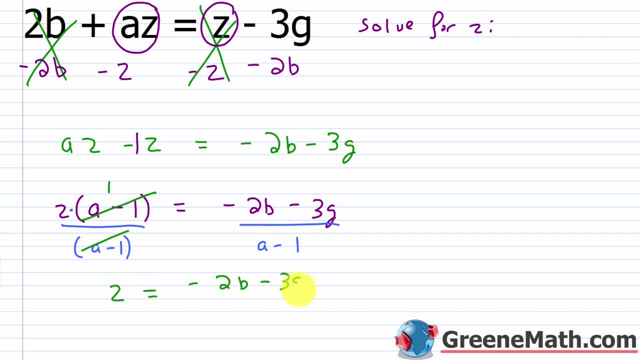 I'll have negative 2B minus 3G over A minus 1.. And that's your answer for Z. So if you get something like that on a test that says solve for Z, that's exactly what you would do. Now you might get different scenarios. You might have a problem that says: 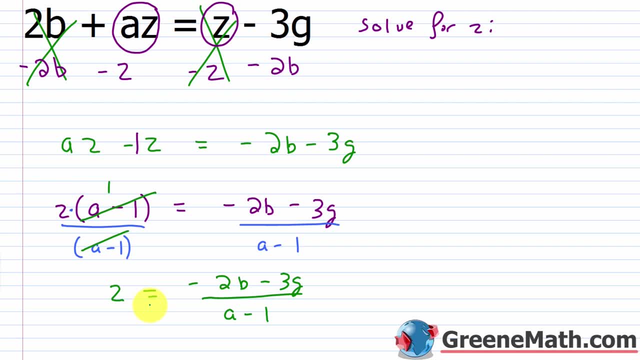 solve for Z, Solve for A, Solve for B, Solve for G, You might have to solve for each one. In the end, you're just going to isolate whatever they want you to solve for on one side of the equation and everything else is on the other. 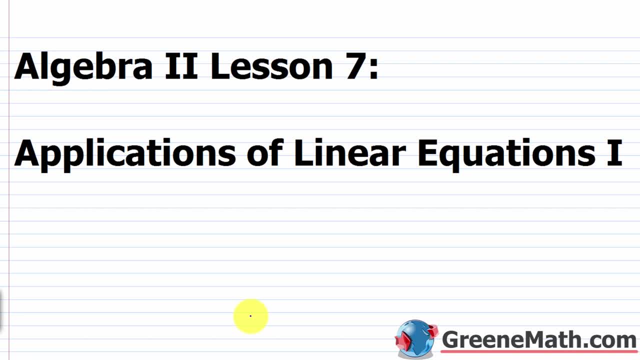 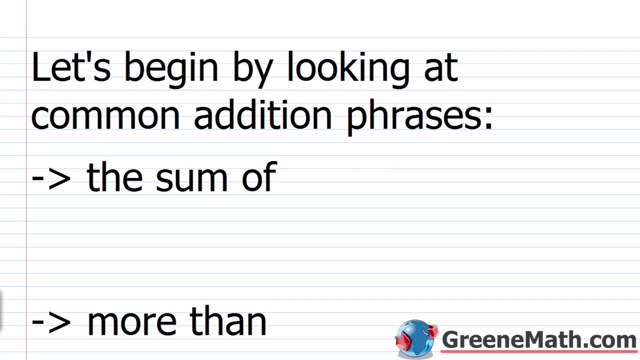 Hello and welcome to Algebra 2, Lesson 7.. In this video we're going to have an introduction to applications of linear equations. So one of the most difficult things you're going to do in an Algebra 1 and Algebra 2 or even a college Algebra course is learn how to 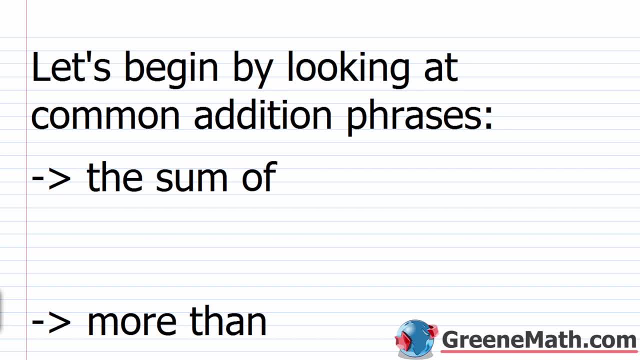 set up and solve word problems. I know if you've done them in Algebra 1. it's something where a lot of students just struggle because you have to generate your own equation before you even struggle to solve it. But one of the things that can help us if we just start out with 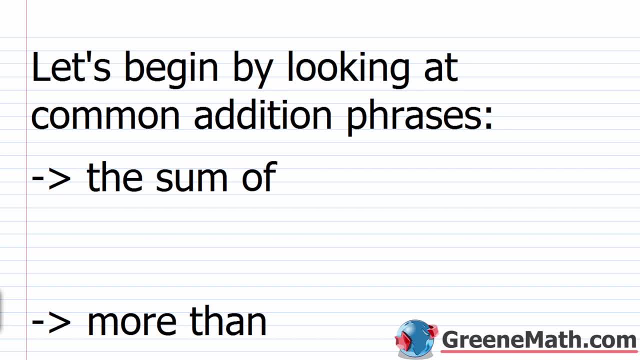 some very, very easy problems and we learn how to correctly interpret some of the language that we're going to encounter with a word problem. I think it's going to put us a step ahead when we start seeing stuff that's very challenging. So let's begin by looking at 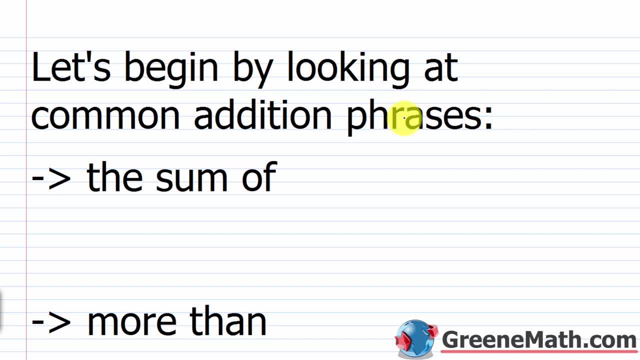 common addition phrases, and then we'll move into subtraction and multiplication and division. So the first one I have here is the sum of. So it's obviously telling us to add. We know the sum is a result of adding. So if I see something like the sum, 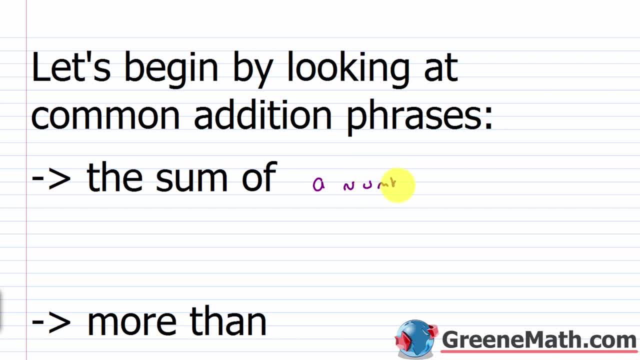 of, let's say, a number and five. How could I represent that? Well, a number is just some unknown number and we can use a variable like x or y or whatever you want to use to represent that. So if I re-read this as the sum of 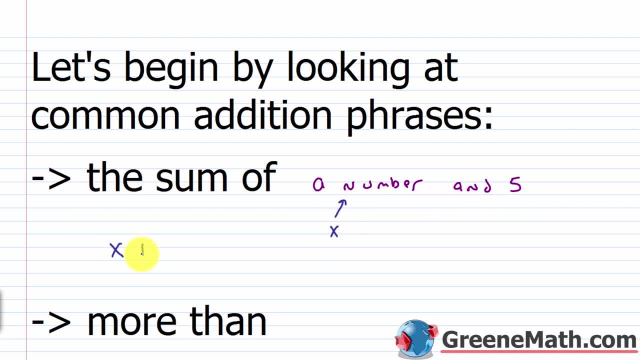 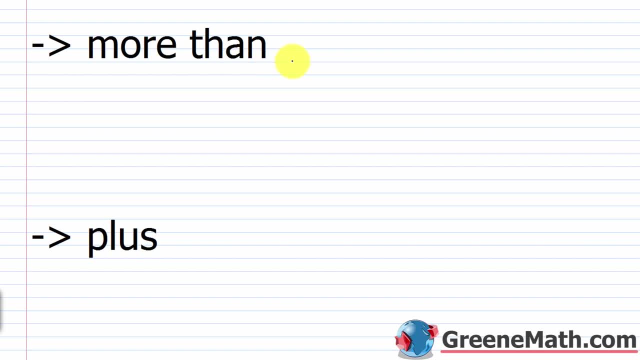 x and five, that would be x plus five. Then you have something like more than. If I saw a phrase that said three more than a number, So let's say I saw three more than a number. And again when we see a number, we can use a variable. Let's use y this time to represent. 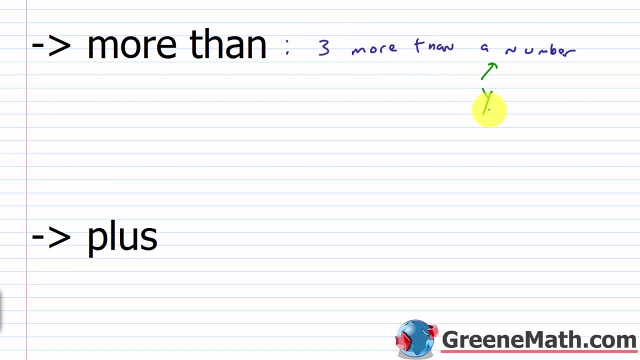 that. So if I saw three more than y, that's just y plus three or three plus y. Remember, addition is commutative, So when you translate stuff with addition the order is not important. So I could put three plus y or y plus three. 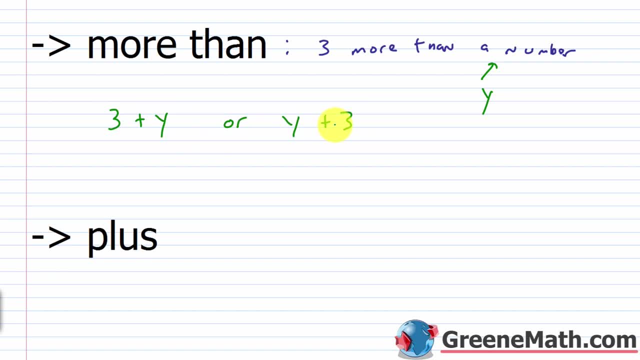 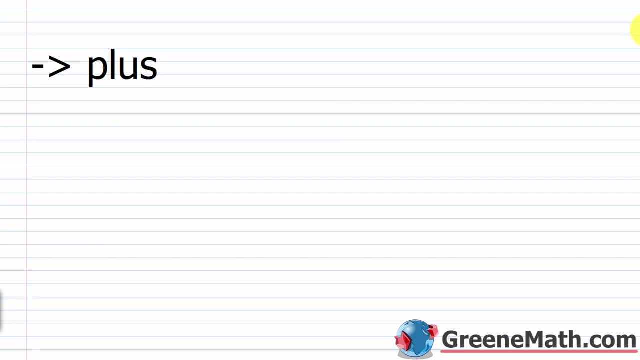 and it's completely irrelevant, because I would have the same answer either way. What about just plus, The plus that we often hear with addition? Well, I could say something like negative seven plus a number. So I could say negative seven plus a number. 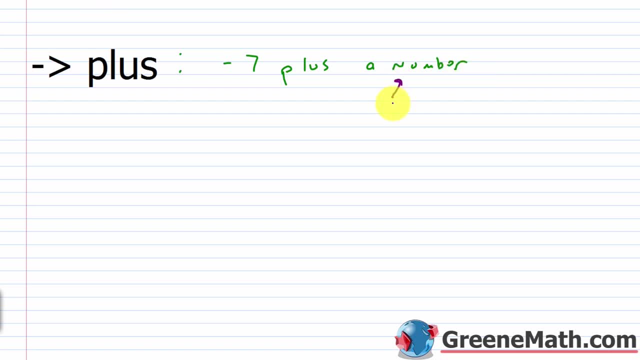 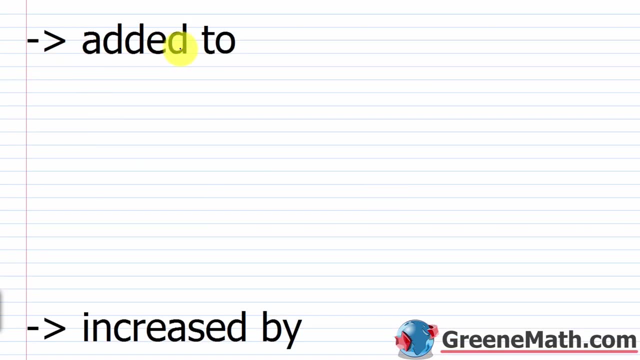 Let's use z to represent a number, So I would have negative seven plus z. Then we also see something like added two. So if I said a number added to negative two, So let's do a number added to negative two, What would that be? 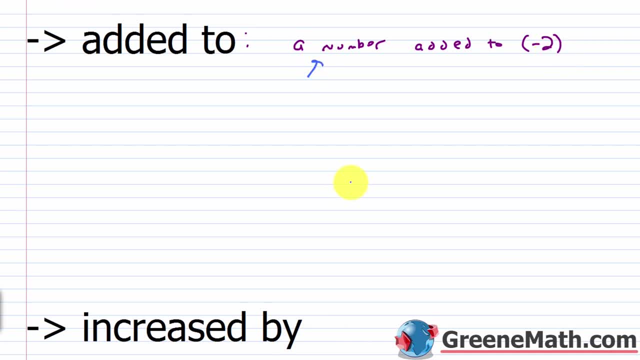 Well, I can use again a variable to represent a number. Let's use- I don't know- q, for example. So if I said q added to negative two, Then I would have q plus negative two. Or again, I could put negative two plus q. 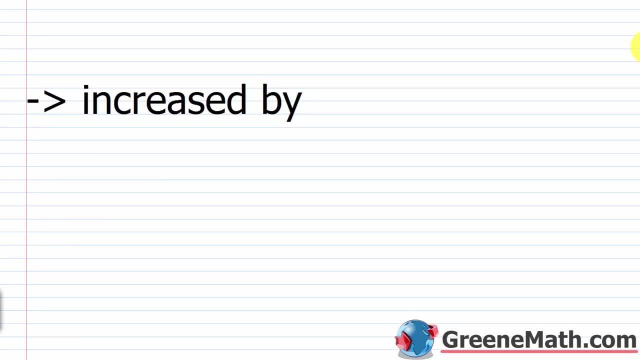 Again, addition is commutative, so the order is not important. What about something like increased by? If I saw a number increased by seventeen, So a number increased by, let's say, seventeen. Well, again a number. Let's use r in this example. 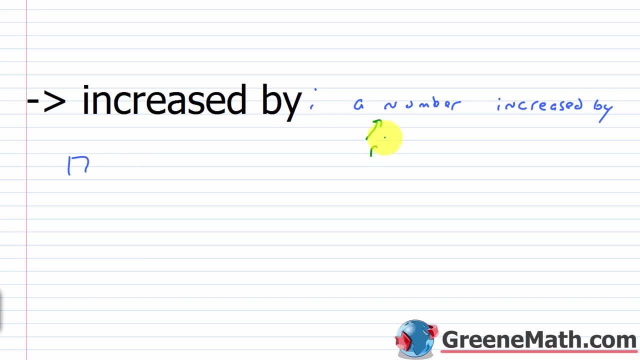 So let's say r increased by seventeen, So we just have r and then if I'm increasing it, I'm adding. So I'm just adding what it's increased by, which is seventeen. So this is r plus seventeen. So you can see, with addition it's very, very easy. The translation is straight forward And remember. 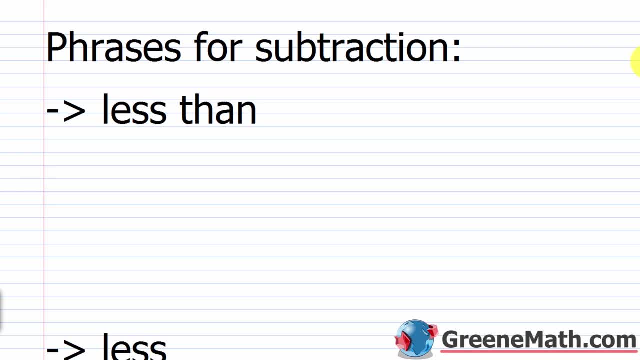 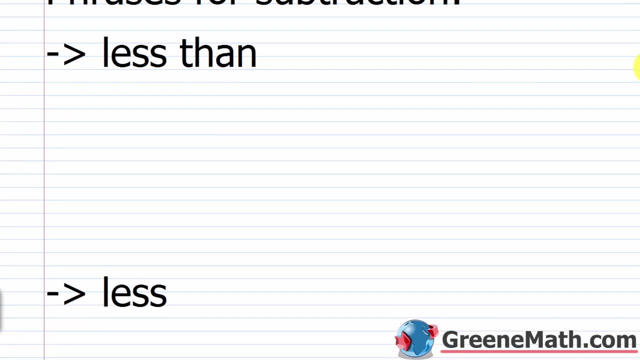 when you're adding things, the order is not important. So let's talk a little bit about some phrases for subtraction. So we have less than. So let me scroll down a little bit. For less than, let's use the example of six less than a number. 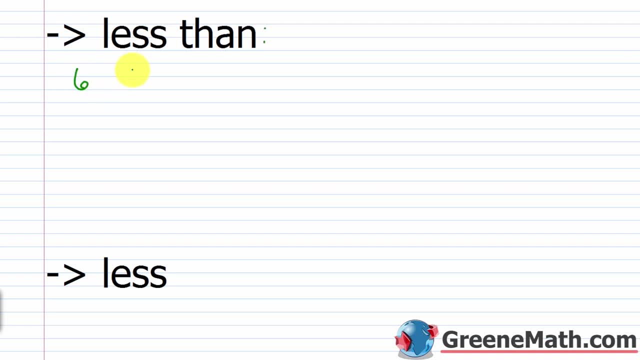 So let's put six less than a number, And I want you to pause the video for a second. Let's just use x to represent a number And when you pause the video, I want you to try to write this phrase Now, hopefully you tried this And I want to walk you through this real fast. 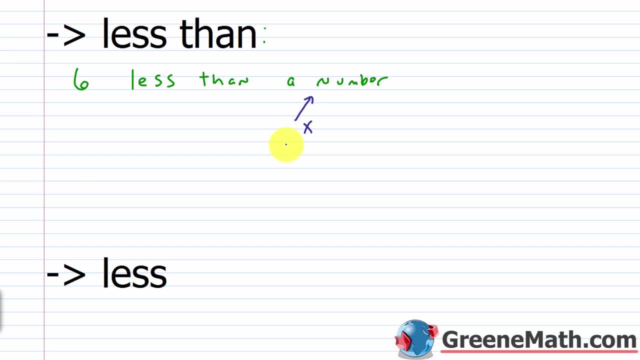 Six less than a number. So that means I have some number and I represented that with x And I want six less than that. So I start out with this and I subtract away six. Okay, If I put six minus x, that would be wrong. This is wrong. 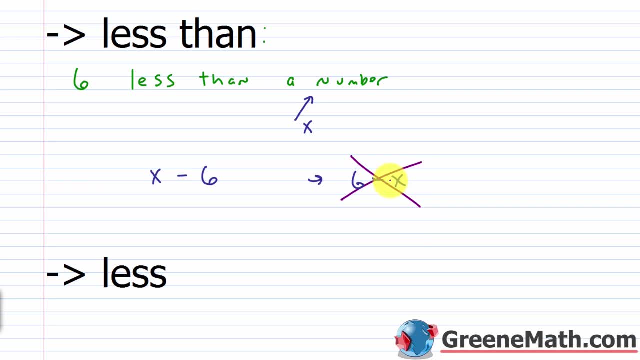 This would be six less a number. Okay, With subtraction. the wording is important. Okay, Because subtraction is not commutative. If I have one minus two, that's not equal to two minus one. Alright, I can't just flip the order there. It's not like. 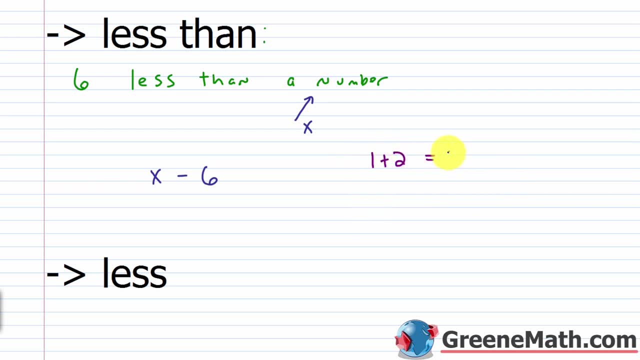 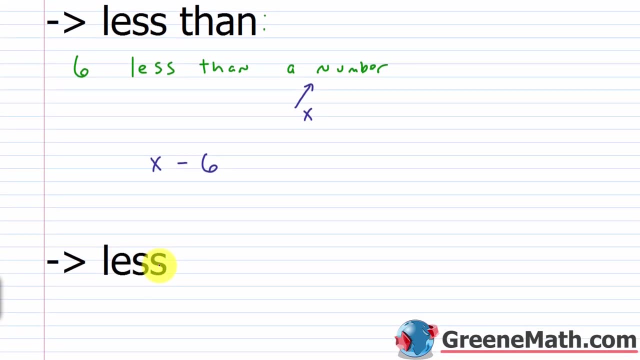 addition, Whereas if I have one plus two, that's the same as two plus one. Okay, Again, subtraction is not commutative. Now on this one where we have less, I can show you. Let's say I had six less a number. 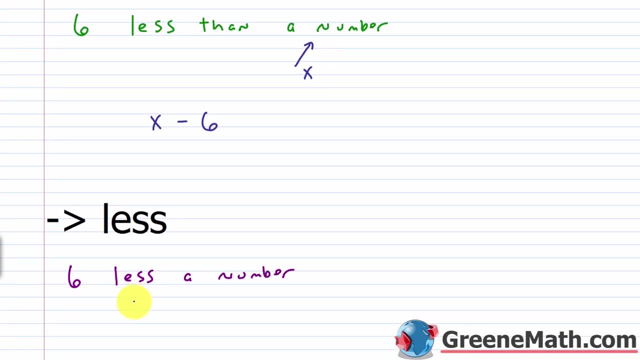 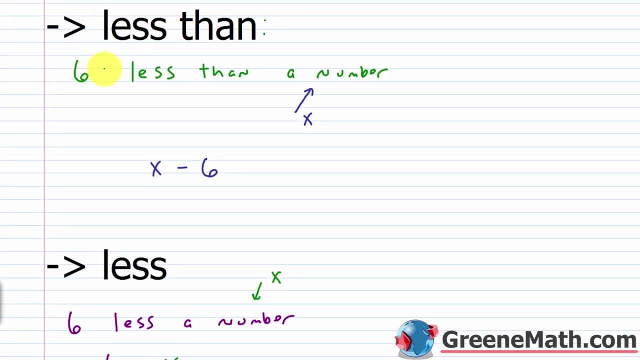 Well, in this case this translates to literally six minus. and then, whatever we use for our variable, in this case, let's use x again. So this is six minus x. So again, notice the difference between the two. In this example we have six, less than a number Implying. 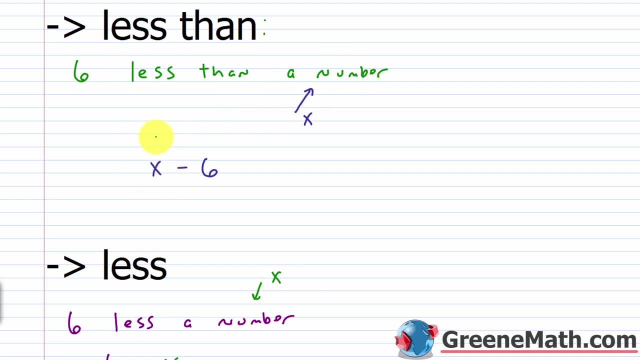 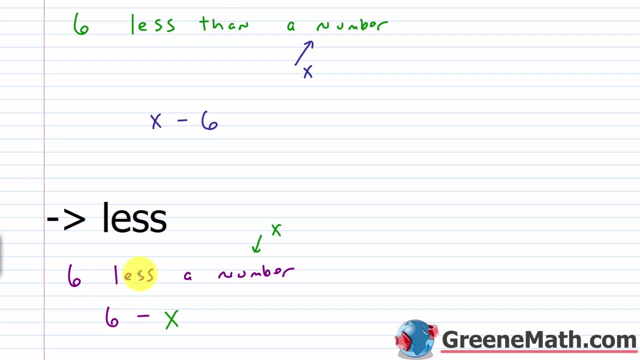 that we start out with the number which is x, And then we're six less than that, so we just subtract away six. In this example it's six less, Just less a number. So six less a number which we represented with x. So again, very important that you understand what you're. 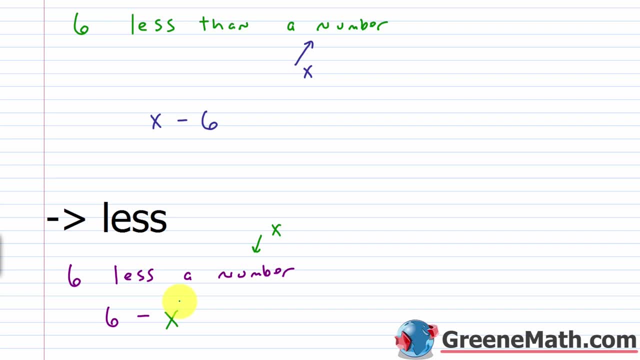 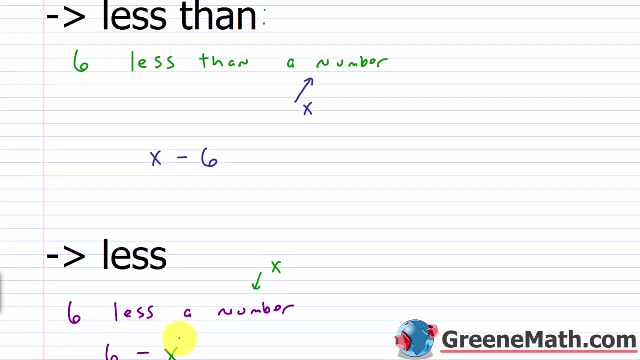 being asked. Take your time when you're reading these things, especially at first, And ensure that you are translating them correctly, because if you don't, most of the time you will get the wrong answer. Alright, so next we see: decreased by. So as an example, let's say I have 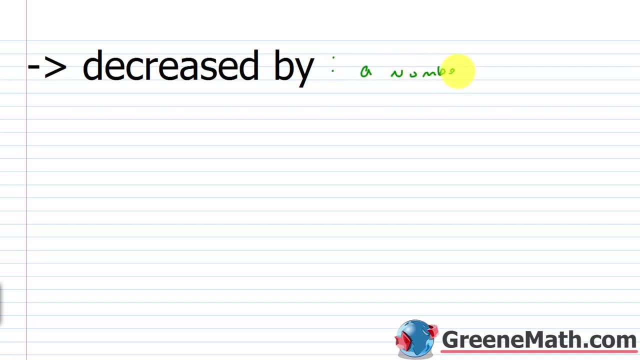 a number. So a number, And it's decreased by, let's say, eight. So let's say the number. here we represent that with y. So y decreased by eight would simply be y, and then it's decreased or we're subtracting away eight. So very, very simple. Then, as another one, let's say we: 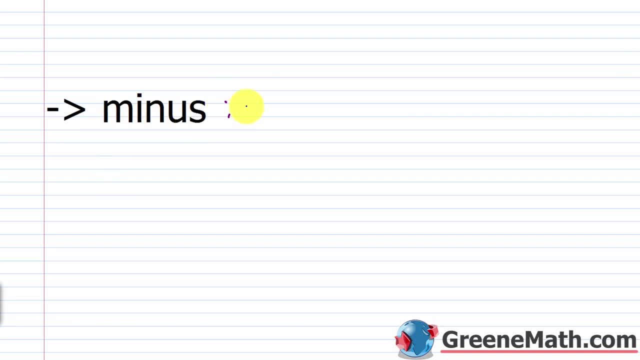 see minus. We know minus means subtract. So let's say I saw four minus a number. Very straight forward. If I use, let's say, z to represent a number, then that's just four minus. okay, minus z. Alright for the last one, for subtraction, let's look at: 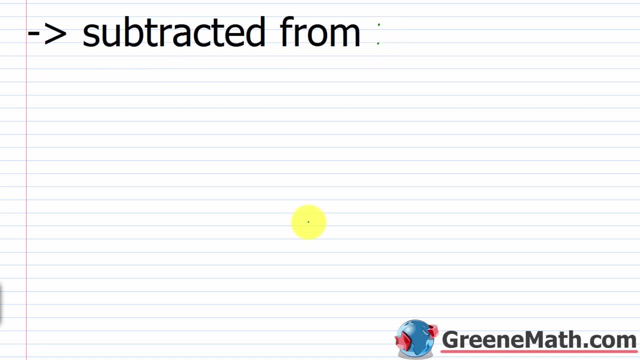 subtracted from. So let's say, as an example: I say a number, So a number Subtracted from I don't know. let's say eleven, So a number. let's represent that with I don't know. let's go with q again. 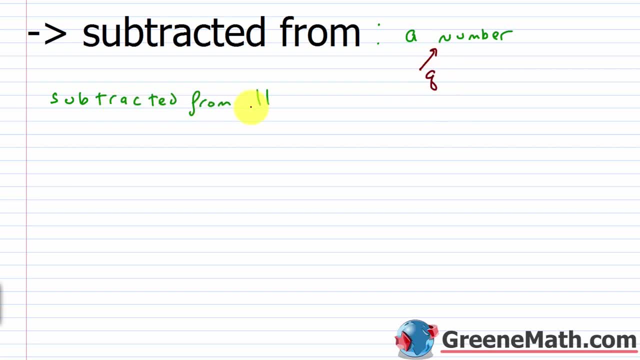 So let's say q subtracted from eleven. So if it's subtracted from eleven, that means I'm starting out with eleven and from that I'm subtracting this number, q, So that's eleven minus q. And again, this is one of those ones where it's very easy to make a mistake. If you put 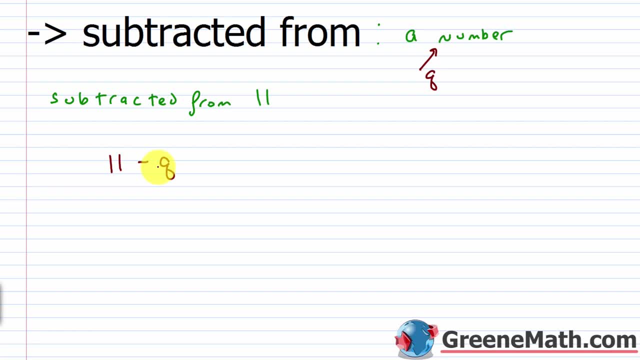 q minus eleven. again, that's not going to be right. You need to make sure that you translate this as q subtracted from. This is the key thing here: It's subtracted from eleven. So that means I have eleven and then I'm subtracting away. 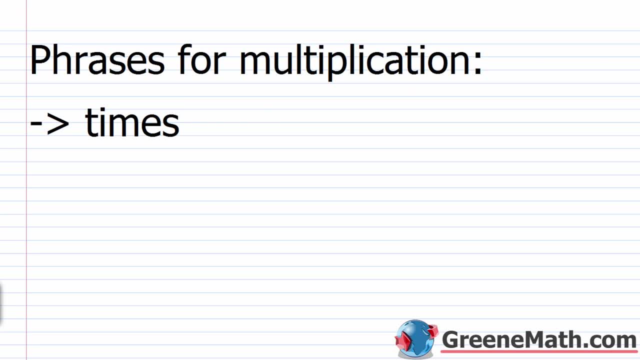 q. Alright, so now let's look at multiplication and with the phrases for multiplication. again, Multiplication and addition are commutative, so we're not going to have the same issue with subtraction. If I have six times three, that's the same as three times six. 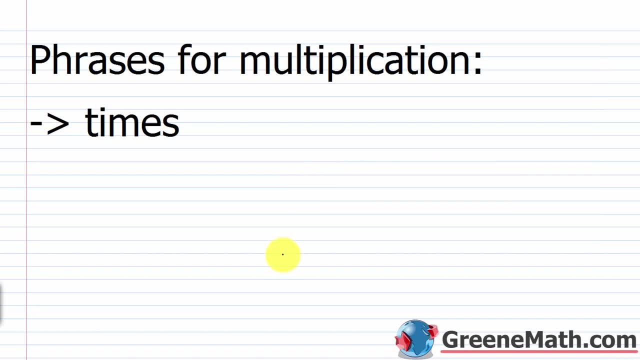 So the order with multiplication is not important. So we start out with something very simple like times. So if I have, let's say, nine times a number And with a number, I can just represent that with, let's say, x again. So nine times x would just be nine x. 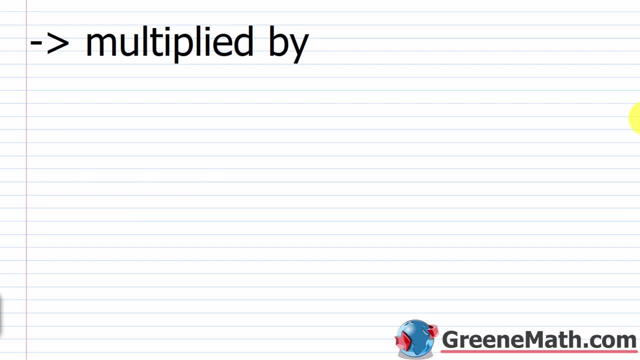 The next one is also obvious. You have multiplied by. So if you saw something like a number multiplied by, let's say, negative seven With a number, I could represent that with anything. Let's say r. So let's say r multiplied by negative seven, That's negative seven times r. 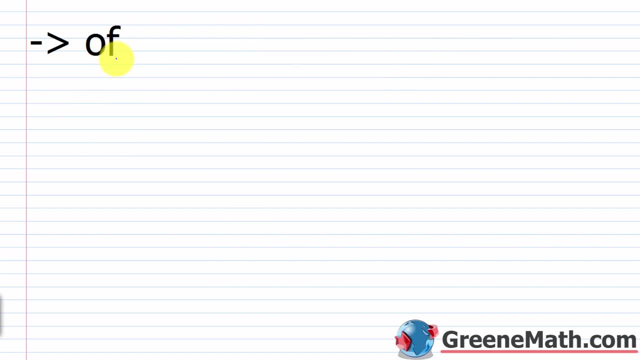 which we write negative seven r. Next, we see of, And we generally see of. when we're talking about fractions, You might see something that says one third of a number, So of let's put one third of a number And let's represent a number. 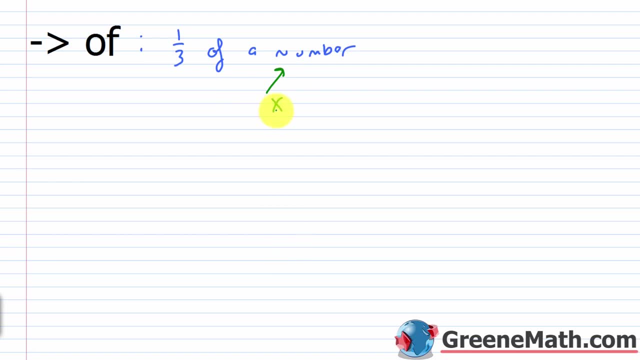 with. let's go with x again. So one third of x just means one third x. It'd be like if your paycheck was three dollars and I said, give me one third of your three dollars, I would get a dollar Alright. the last one we're going to look at with multiplication is product. 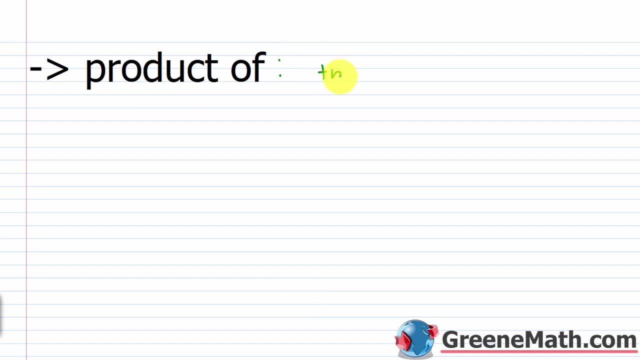 of, And for this one we could just say the product of a number and let's say negative fifteen. So the product of a number which I'll represent with, let's say, y and negative fifteen would be negative fifteen times y or just negative fifteen y, Alright. lastly, let's look at some phrases for division Again. 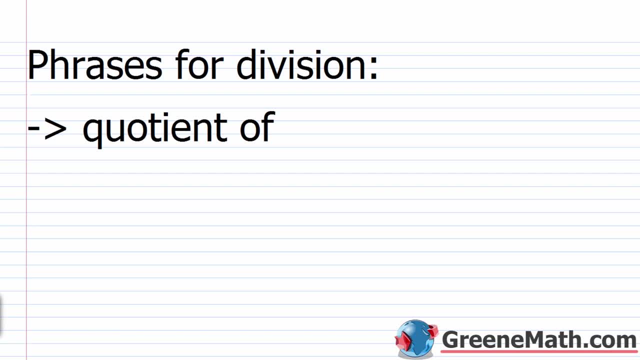 remember, division is also not commutative. If I have you know, ten over two that's not the same as two over ten. These are not equal to each other. So when we look at phrases for division, we start out with the quotient of. So let's. 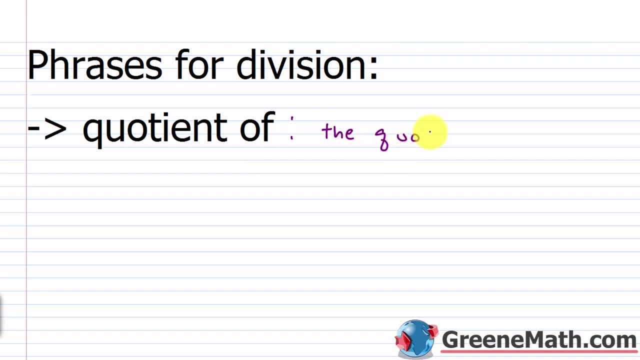 say: I have the quotient of seven and a number. So this would tell me that I have the quotient of seven. Seven is going to be the numerator and a number A number is going to be in the denominator and I'll represent a number with just x. So this: 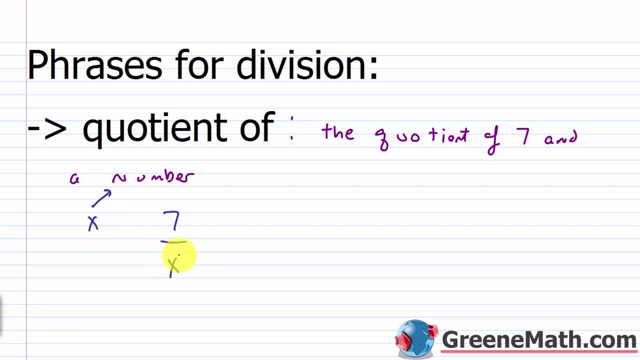 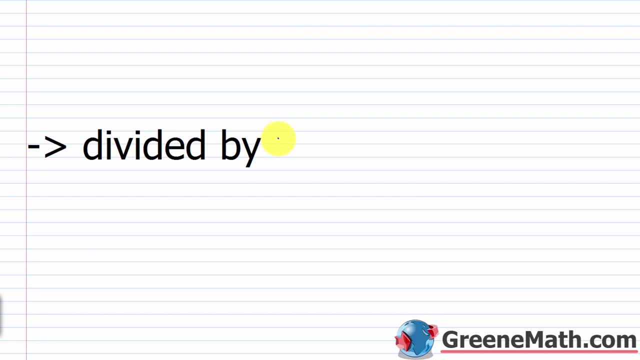 would translate into seven over x, The other one we really see with division. a lot is divided by, which obviously makes sense, And you see something like a number divided by, let's say, negative two. Now a number. let's represent this with z. So a number, so z divided by negative two. 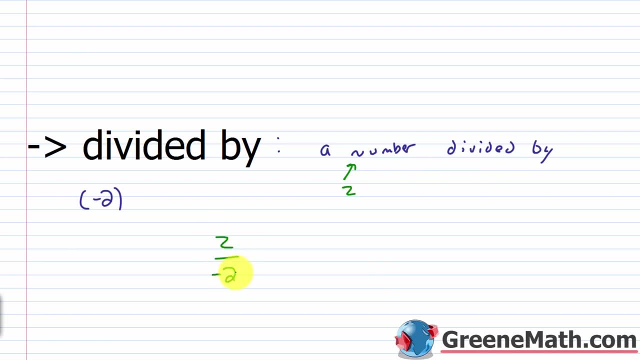 would just be z over negative. two And again, when you encounter phrases with subtraction and division, you have to be extra careful to read your wording and interpret it correctly. Alright, so the last thing we want to know before we start looking at some problems is means. 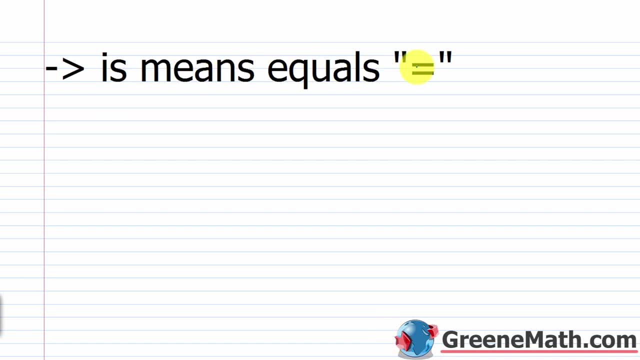 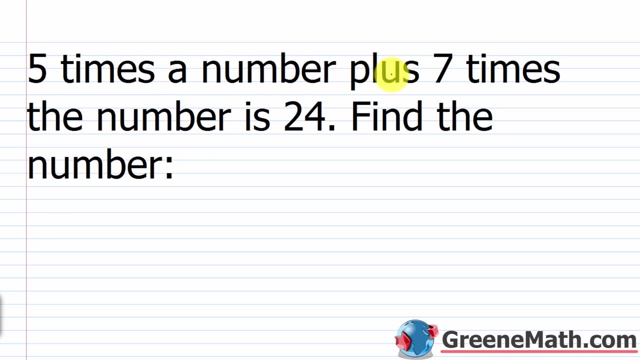 equals. So that's the translation when we're looking at a word problem. Alright, so let's look at some sample problems. So here's the first one. We have five times a number plus seven times the number is twenty-four. Find the number. 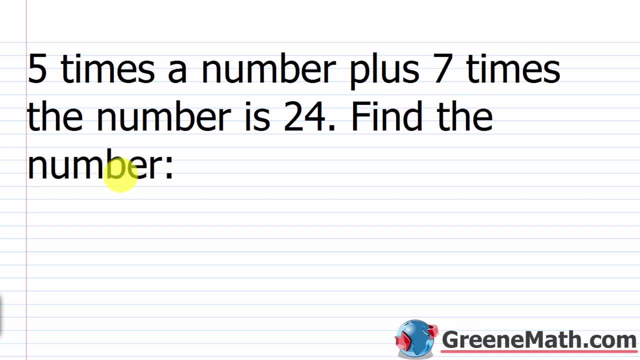 So the first thing I like to do when I encounter these is: I represent a number or the number or whatever it is that's unknown with a variable. So let's line this out and just put x there. Let's line this out and just put x there. 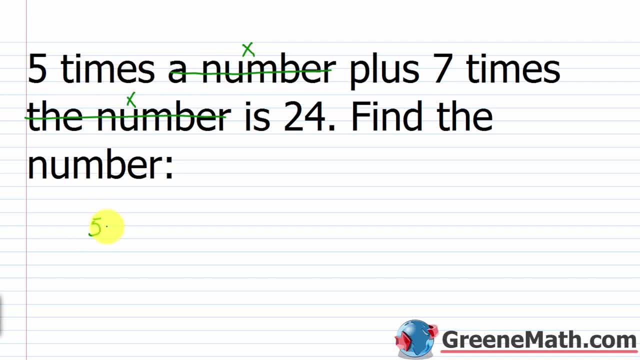 So five times x is five, x plus means to add. seven times x is means equals, and then twenty-four. Very, very simple once you do that. So I've just translated this to this And now that I have an equation, it's very, very easy to solve and find. 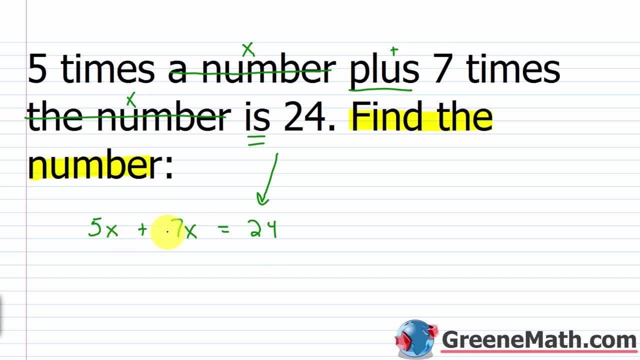 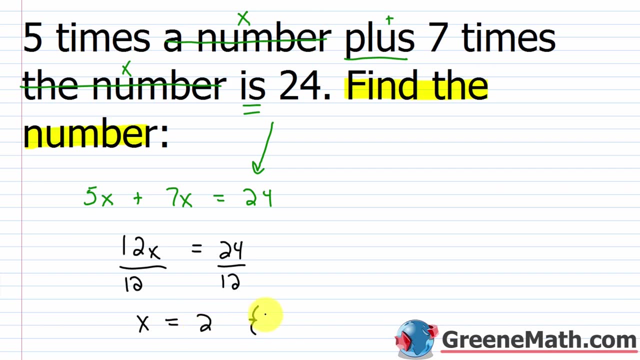 the number. So five x plus seven x. we combine like terms there we get twelve x and this equals twenty-four. We divide both sides of the equation by twelve and we get that x is equal to two. or again, using solution set notation, we say that this set contains the element two. 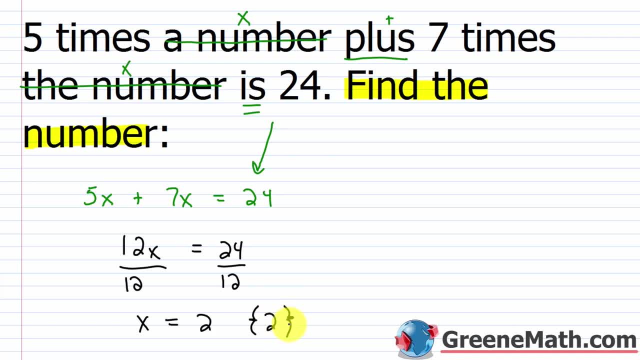 Now, when you solve a word problem, you generally want to answer with a nice little neat sentence. So we can just make something really simple and say: the number is two, Or we can just put the number is two, like this. Either way, Alright, let's take a look at another one. So we have a number. 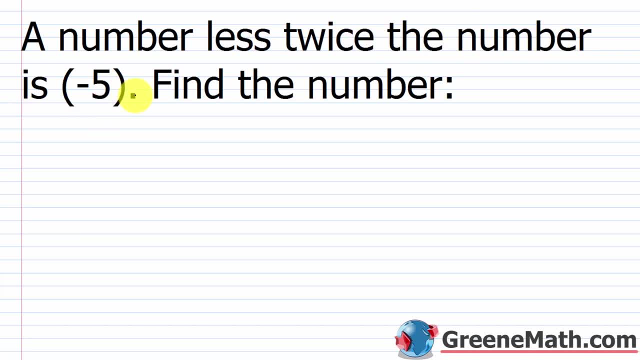 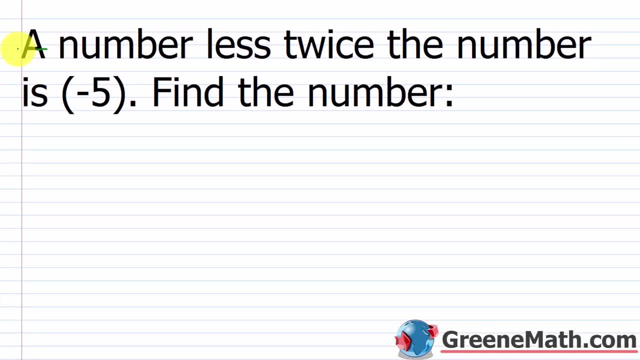 less twice the number is negative five, Find the number. So again, everywhere I see something like that. I'm going to replace it. So let's just line this out and put x or y or z or whatever you want to use. So x less. 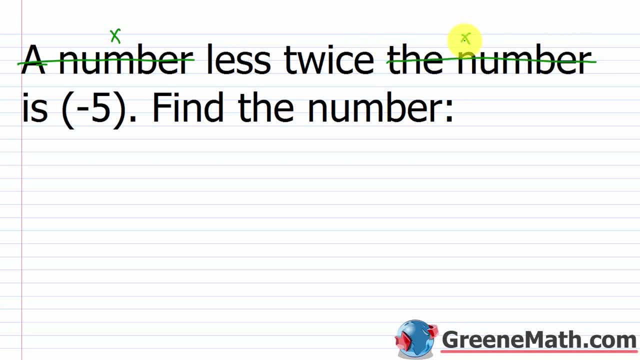 twice the number. so let's line this out and put: x is negative five, So let's put equals here. Okay, So now I have x less, So I know that that means I have x, and then I'm subtracting away because I see less. 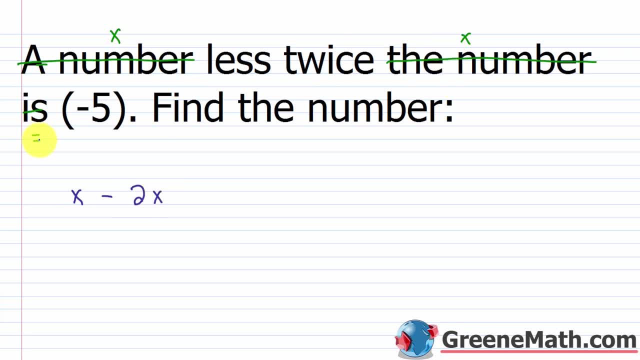 Twice x, so that's two times x, and then equals for is negative five Again. once you kind of label things like this, it's very easy to go from this to this: Okay, So now I have x minus two x. that's negative x. 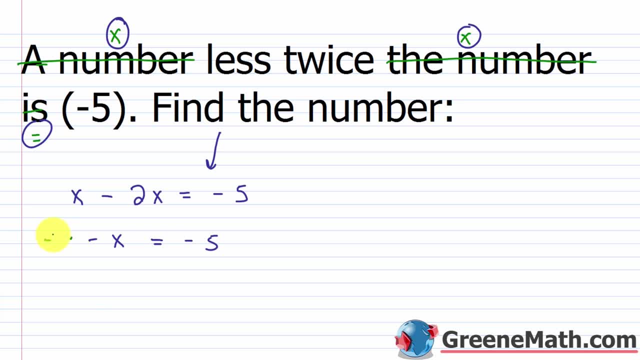 This equals negative five. If I multiply both sides of the equation by negative one or divide by negative one, whatever you want to do there, This cancels with this and I have: x is equal to negative. five times negative one is five. So find the number, The number. 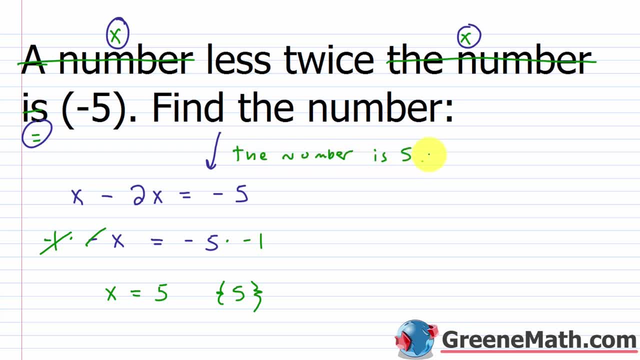 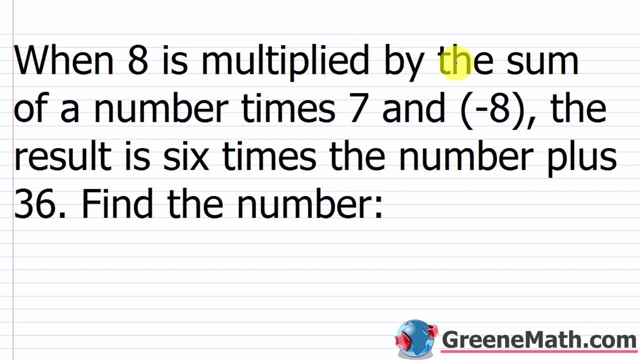 is five. Okay, let's look at one that's a little bit more complicated now. So when eight is multiplied by the sum of, and then we have a number times seven and negative eight, The result is we have six times the number plus thirty six. 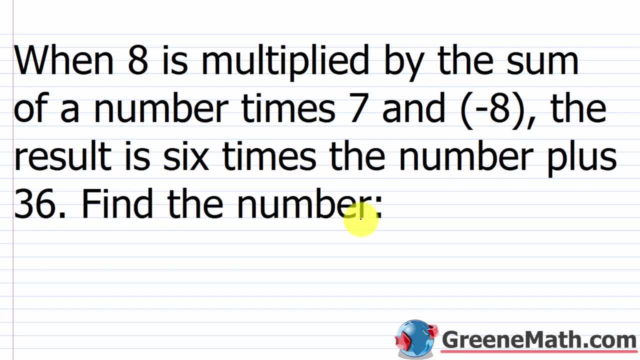 and then we just want to find the number. There's a few things in here that can really trip you up if you've never done any of these problems. So the first thing is that we're going to be using our distributive property here. I want you to. 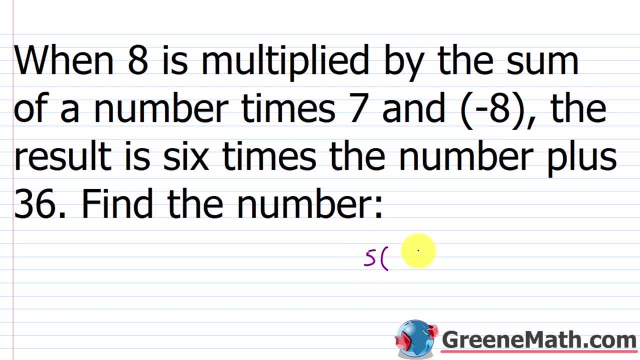 recall. if I have something like five times, Let's say I just write two plus three, like this, I would do five times two plus five times three and that gives me ten plus fifteen, which equals twenty five. I know that if I combine two and 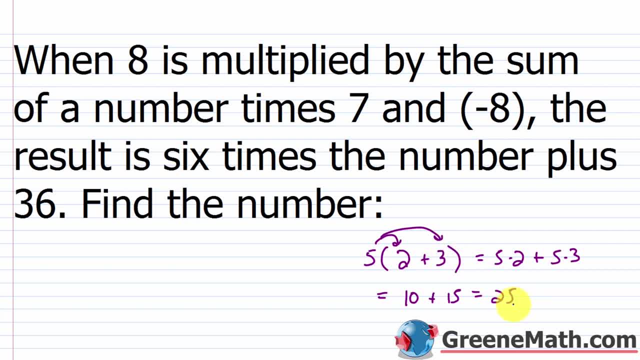 three. through addition, I'd have five. Five times five is twenty five. In the case where we have a variable involved, we know that we could say we have the sum of, let's say, two x plus three. Now I can't combine these because they're not like terms. So in this case I do five. 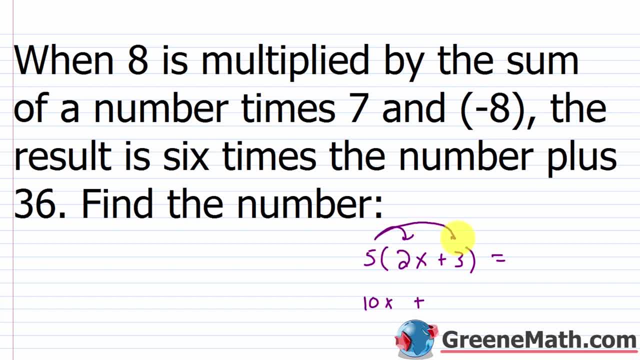 times two x, and I get ten x plus five times three, which is fifteen. So if I had told you I have five times the sum of two x plus three, you would have to write it this way, because five has to be multiplied by the two x and the three. I can't just write it like this. 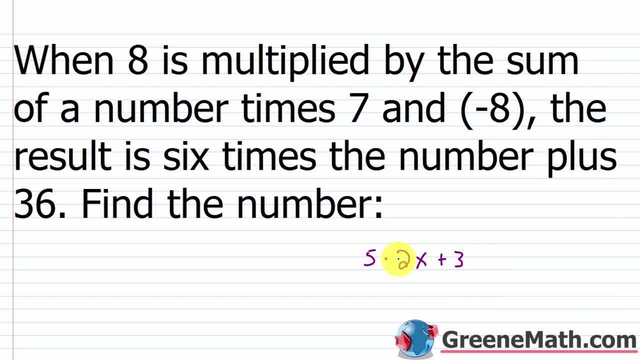 which is a common mistake. Now I'm just multiplying five times two x. I'm forgetting about the three. So it's important you understand that before we start trying to attack this problem. So again, when eight is multiplied by the sum of a number, and I'll replace this with: 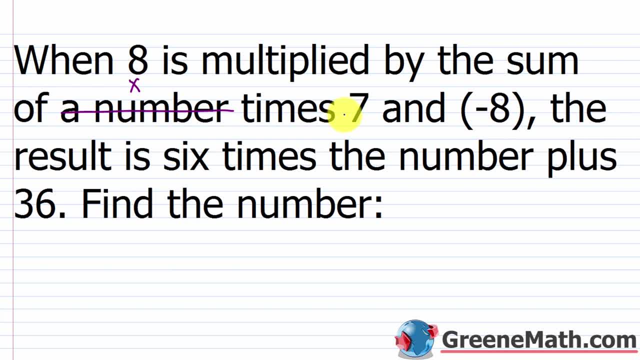 x and it's being multiplied times seven. so this would really be what? Let's just write this whole thing as seven x Makes it nice and simple. So let me re-read: When eight is multiplied by the sum of seven x and negative eight, So eight is multiplied by. 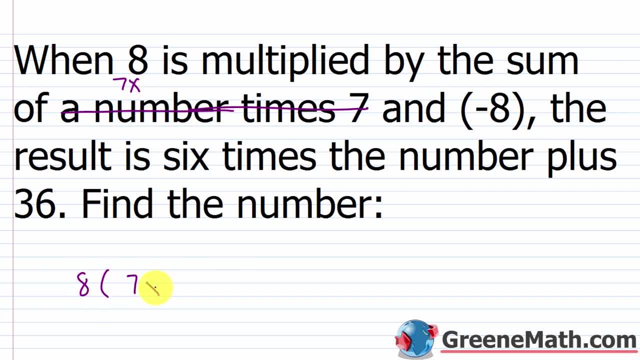 the sum of seven x and negative eight, Seven x plus negative eight or seven x minus eight. But it's important that eight be multiplied by seven x and also negative eight, which is why I used parentheses here- Very important- Just like what I just did over there. Alright, so once we get past that, we say: 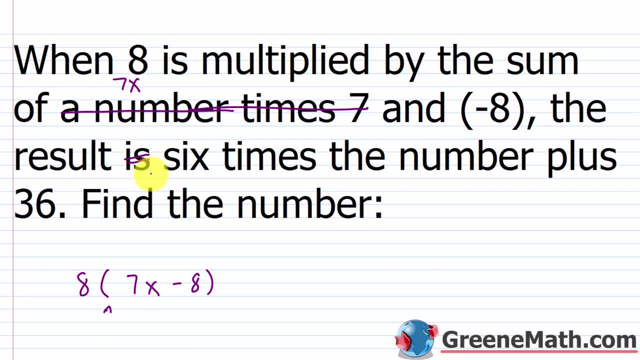 the result is: is, so that means equals. and then we have six times the number. we represented the number or a number with x. so we have six times x, which is six x, then plus thirty six. So again, once you start doing this, enough, you'll recognize. 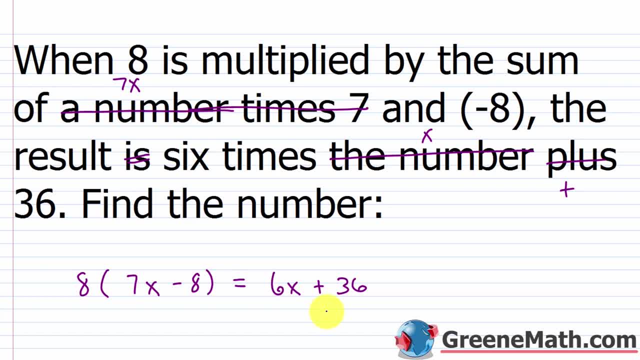 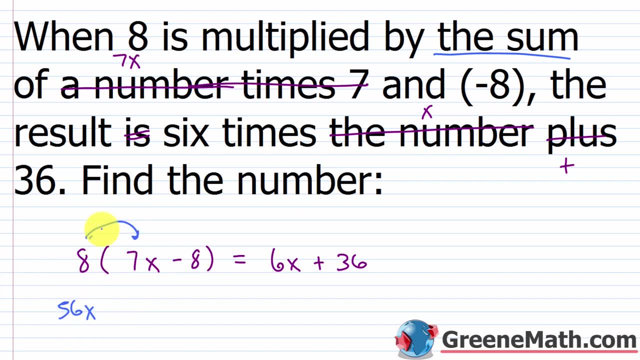 what's going on and you'll be able to translate these very quickly. The key trap here would not be putting parentheses around the sum of seven x and negative eight. Alright, so seven x minus eight. So eight times seven x is fifty six x. and then eight times negative eight is minus sixty four. 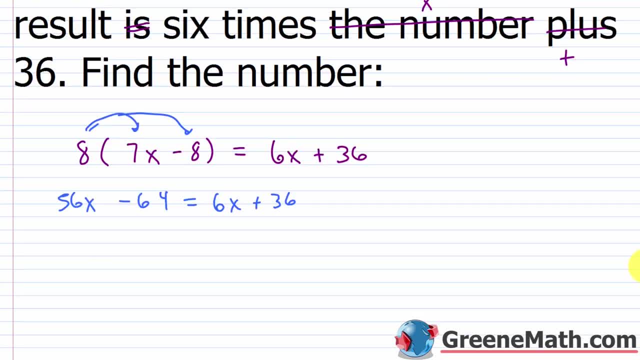 we have this equals six x plus thirty six. So now I want all my variable terms on one side, all my numbers on the other. so minus six x, minus six x plus sixty four plus sixty four, So this will cancel, and this will cancel, so we'll have fifty. x is equal to: 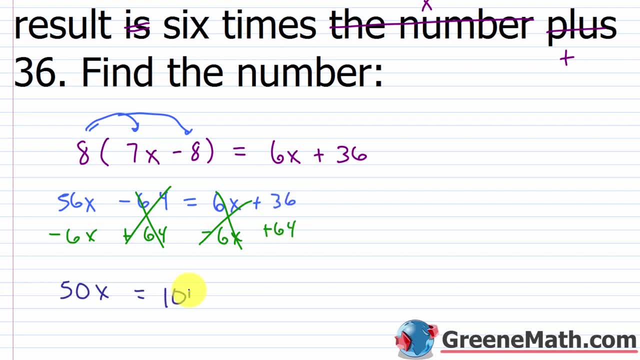 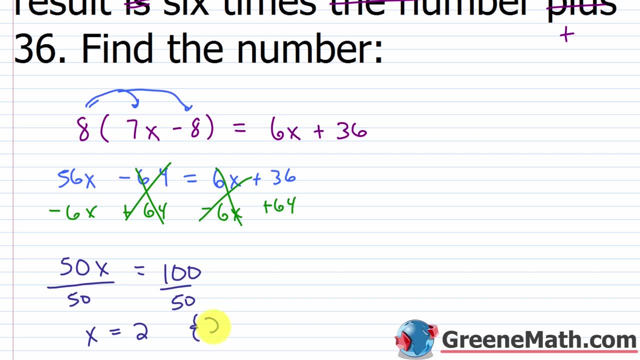 thirty six plus sixty four is going to give us a hundred. we divide both sides of the equation by fifty and we get x is equal to two. So when we answer this, find the number Again, we can just say the number is two. Alright, let's take a look at one. 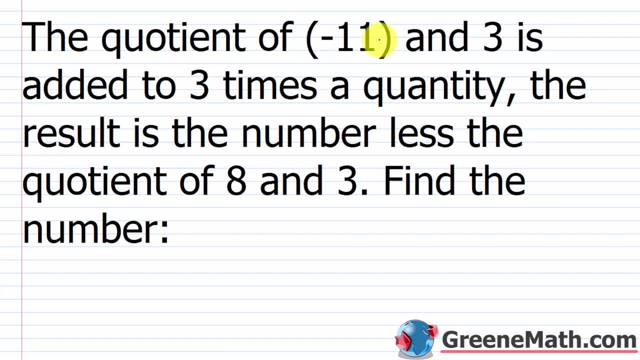 more problem. So the quotient of negative eleven and three is added to three times a quantity. The result is the number less the quotient of eight and three. Find the number Again. these seem kind of difficult, they seem kind of really wordy, but if you go step by step it's not that bad. So the 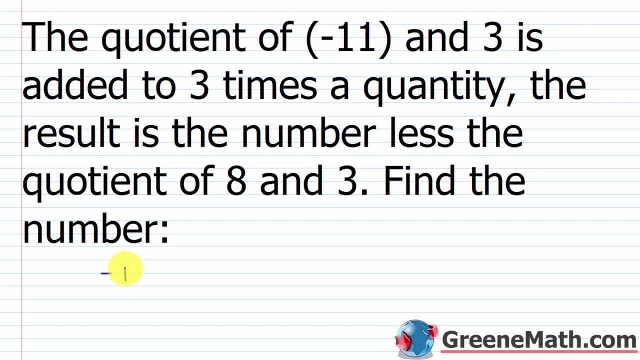 quotient of negative eleven and three. That's negative eleven divided by three. Very simple, So is added two. So is added two just means plus three times a quantity. So what can we say? We can say: a quantity is just x. So three times x is just three x. 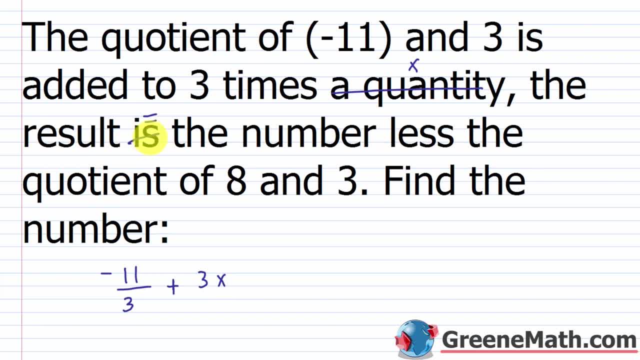 the result is: is means equals the number which we said was x. Then we have less, which means to subtract, so we're subtracting away. Then we have the quotient of eight and three, So that's eight over three. So again, it looks complicated, but once you go step by step, it's really. 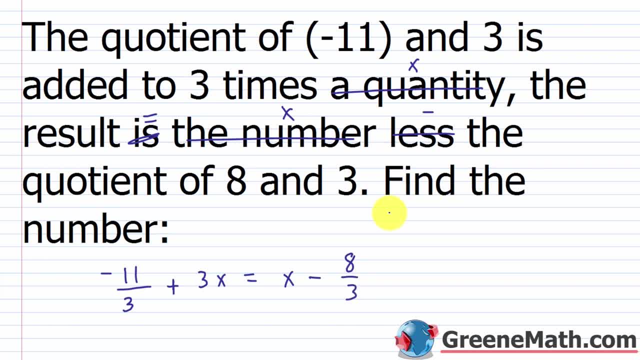 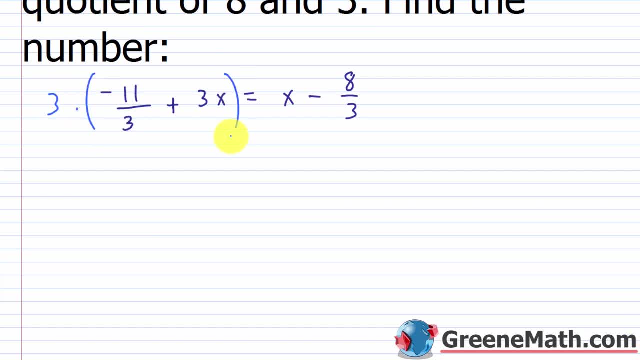 not. So again, we just want to find the number. So let's scroll down a little bit and I'm going to multiply both sides of the equation by three, just so that I don't have a denominator involved. Three times negative: eleven thirds is negative eleven plus three times three x is nine x. 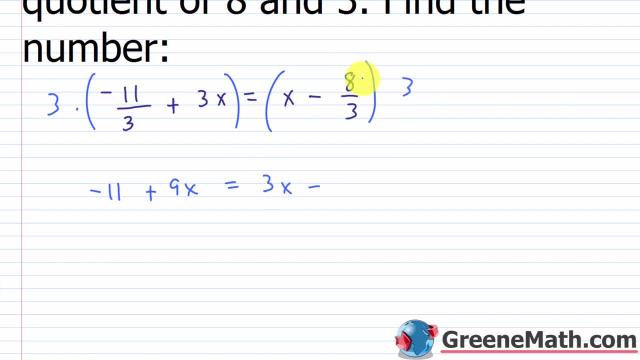 This equals three times x, that's three x minus three times eight. thirds would be eight. Again, I want all my variable terms on one side and all my numbers on the other. So I'm going to add eleven to both sides of the equation. I'm going to subtract three x from both sides of the equation. 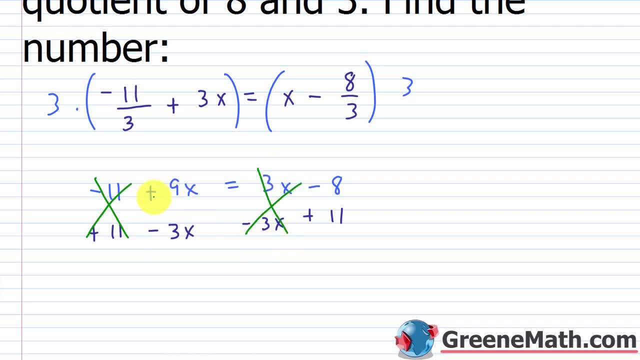 So this is going to cancel, and this is going to cancel. Nine: x minus three, x is six, x Negative eight plus eleven is three. If we divide both sides of the equation by six, we get that x is equal to three over six is basically one half. 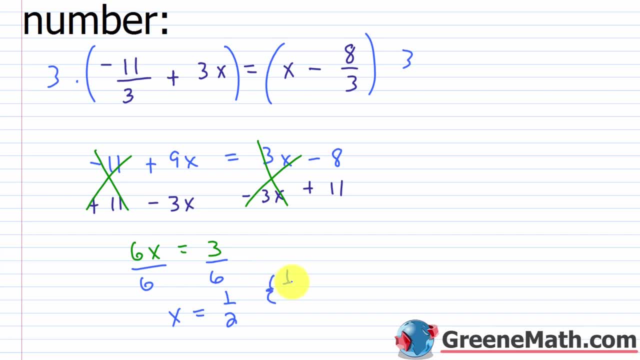 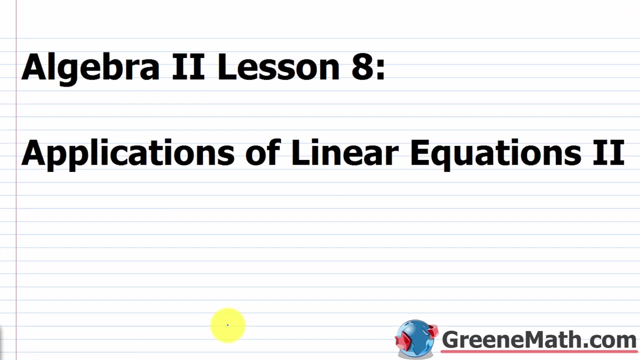 or you could say point five, So the number is one half. Hello and welcome to Algebra 2, Lesson 8.. In this video we're going to continue to learn about applications of linear equations. Alright, so in the last lesson we covered how to translate some basic. 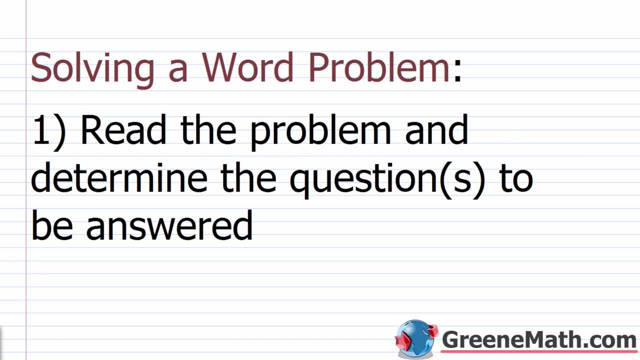 phrases into related mathematical expressions. We then looked at some extremely basic word problems. So here in this lesson we're going to take the next step and we're going to look at some more challenging problems Now, fortunately, most word problems can be broken down into a type. 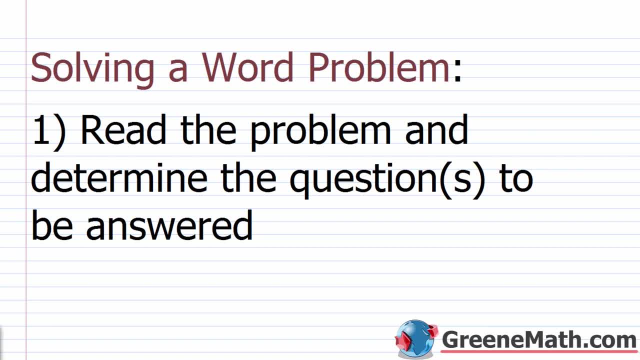 of problem. So in this lesson we're going to look at three different types that you're going to encounter in your Algebra 1 or your Algebra 2 course. So let's begin by looking at a general six step method for solving a word problem. 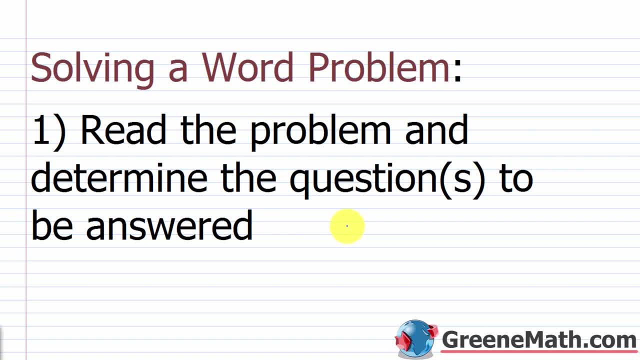 And this method is generally going to pertain to solving a word problem. that involves setting up and solving a linear equation in one variable. Alright, so let's get started with this. So we have solving a word problem. So the first step and the most obvious, 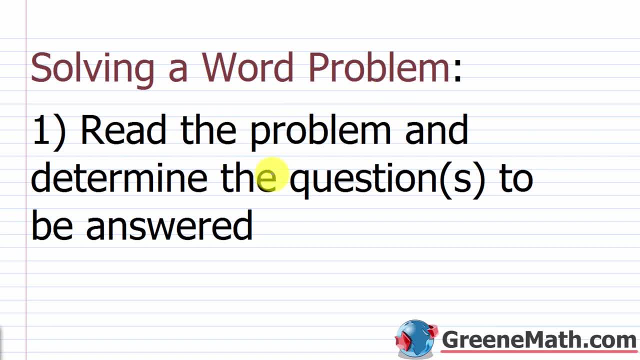 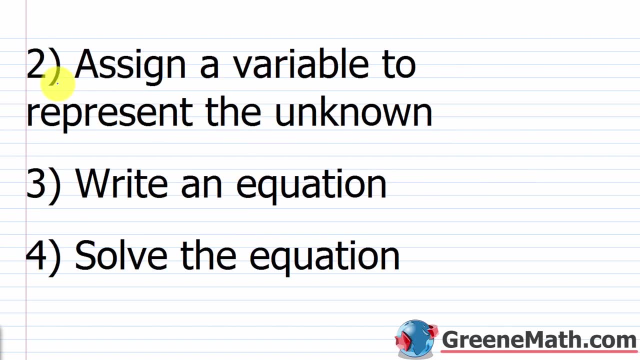 step is just to read the problem and determine the question, or it could be questions to be answered. So it's very important that you take your time and read anything you have extremely thoroughly. Make sure you understand what they're asking you to do. The next step is to assign a variable to represent. 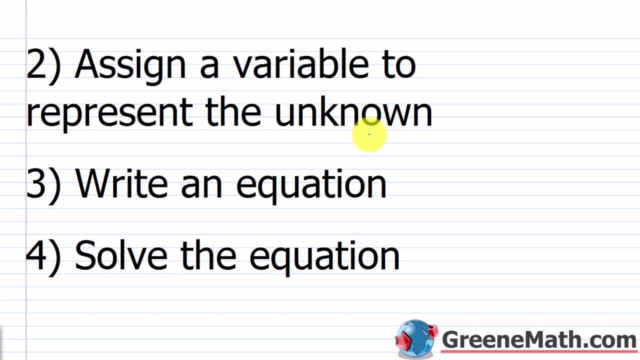 the unknown. Now, in some cases you're going to have more than one unknown. In this scenario, especially when you're in a chapter where you're solving linear equations in one variable, you're going to express any other unknowns in terms of that first unknown that you assigned a. 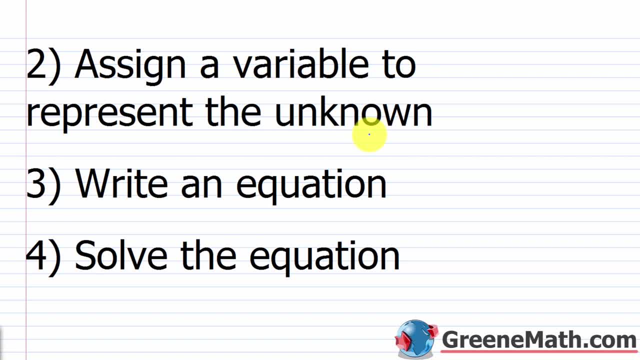 variable to, And that might be a little confusing with me just saying it, but once we get to an example I'll show you what I mean. Now the next step is to write an equation. This can be kind of challenging, especially if you don't have a lot of experience with word problems. 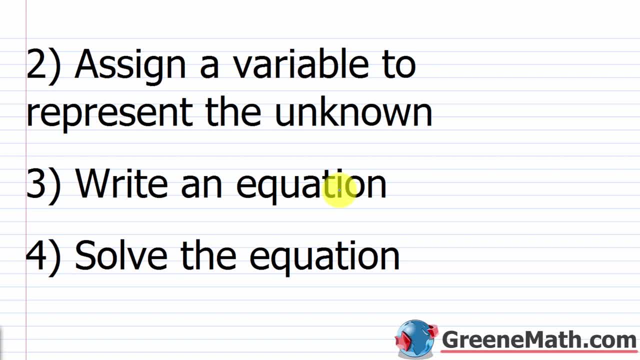 Once you go through and you solve enough problems- especially since the type of problem doesn't vary that much- you're going to get this right away. Then, once you've gotten through this step here, you're pretty much home free. You know how to solve a linear equation in one variable. 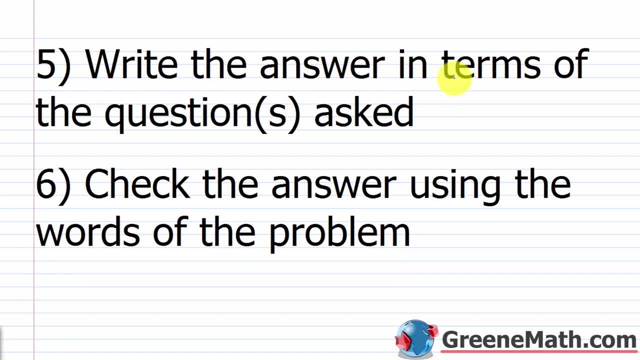 so you're just going to be doing that. Then you're going to write the answer in terms of the question or questions asked, So you make a nice little neat sentence And then the last thing, the most important, is to check the answer using the words. 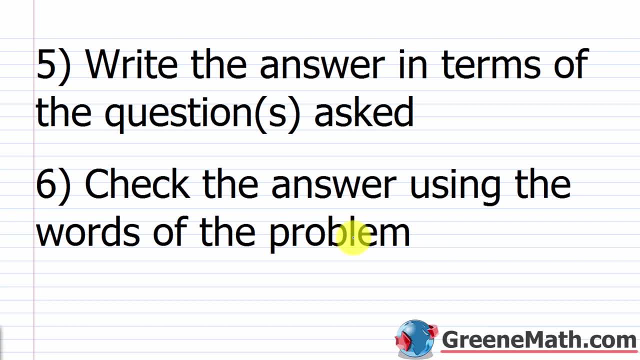 of the problem And you want to make sure that your answer is reasonable. If you got a question that asks how many people are on a bus and your answer is negative 3.7, you know you probably did something wrong. You can't have a negative amount of people on a bus. 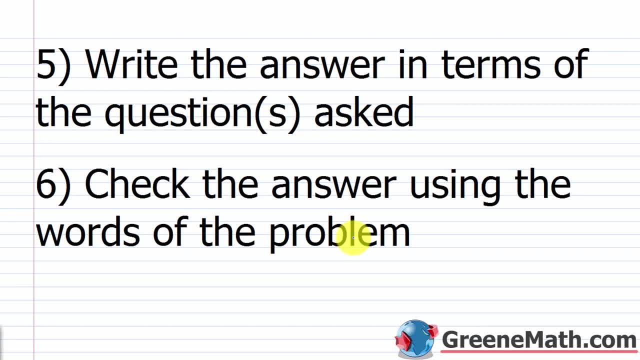 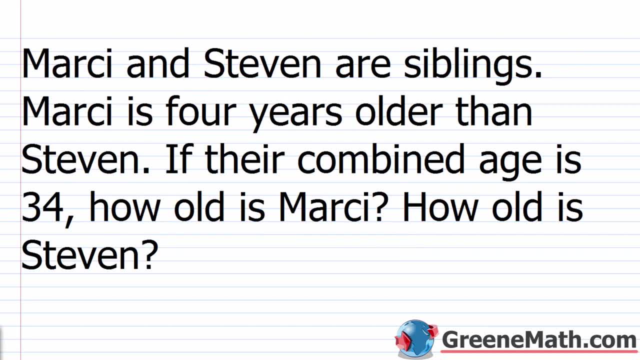 So you want to make sure again that the answer is reasonable in terms of the problem that you were given. Alright, let's go ahead and look at the first example. So this example deals with finding the unknown individual amounts when the sum of those amounts 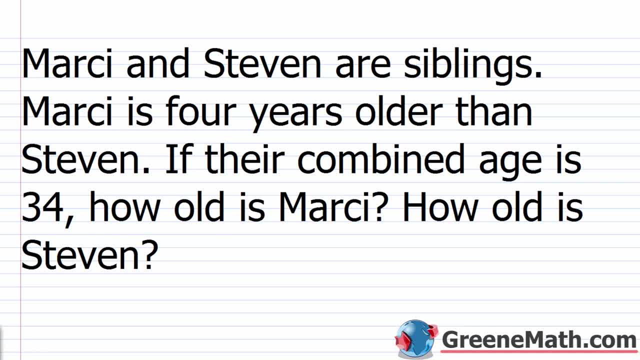 is given. So a very common problem for Algebra 1 and Algebra 2.. So Marcy and Steven are siblings. Marcy is 4 years older than Steven. If their combined age is 34,, how old is Marcy? How old is Steven? 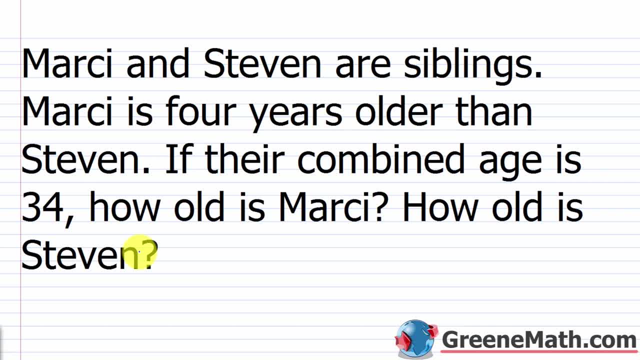 So we've read the problem. I think it's a very simple problem, So most of you will understand that we're being asked to find the age of Marcy and the age of Steven, So that's all we need to find Now. the next thing is to assign a variable to represent. 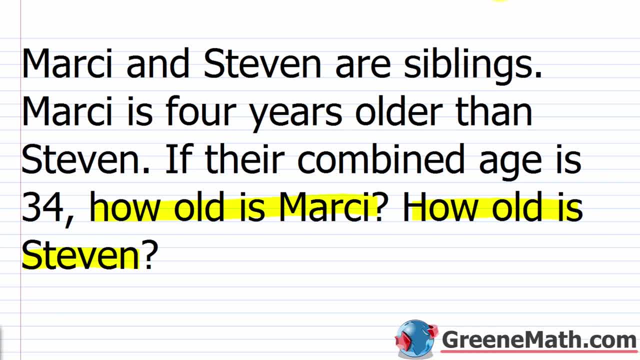 the unknown. Now, in this case again, we have two unknowns. We need to know how old is Marcy and how old is Steven, So I can pick one of those. It doesn't matter which one, And I can let a variable. 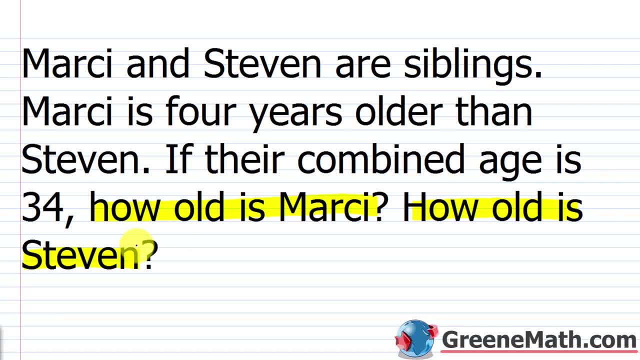 like x, represent their age. So I can just say: let x be equal to. let's go ahead and say Steven's age, Steven's age, And it doesn't matter if I put x equal to Marcy's age or if I put x equal to Steven's age. 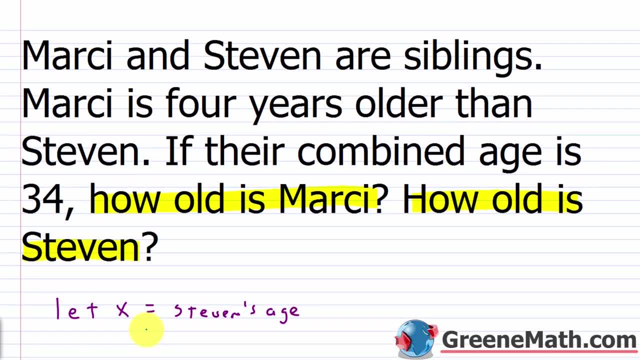 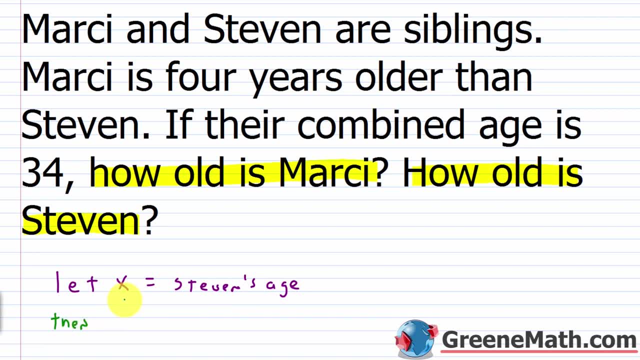 And I'll just do it both ways, just so you can see that it comes out the same way. So if x is equal to Steven's age, then how would we model Marcy's age? Well, we look at the problem again and it says: 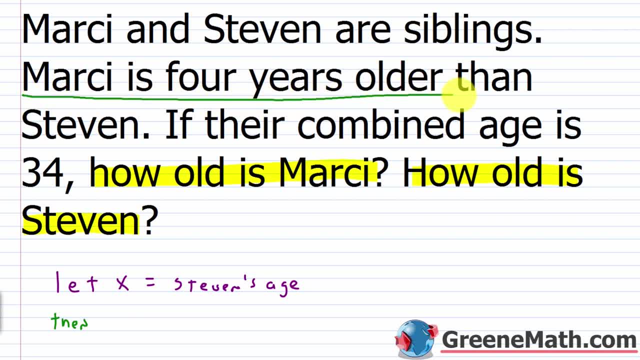 that Marcy is four years older than Steven. So if x represents Steven's age, then x plus four would represent Marcy's age. Now our next step, and probably the most difficult one for us, is to write an equation. So how do I make? 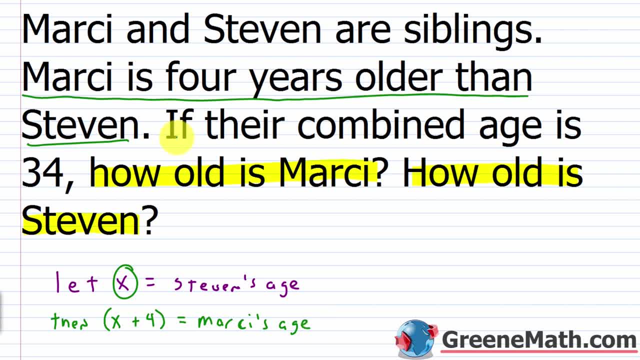 an equation. Well, think about the information you're given. It tells you right here if their combined age is thirty-four. Well, I've represented Steven's age with x. So x, this is Steven's age. And I've represented Marcy's age with. 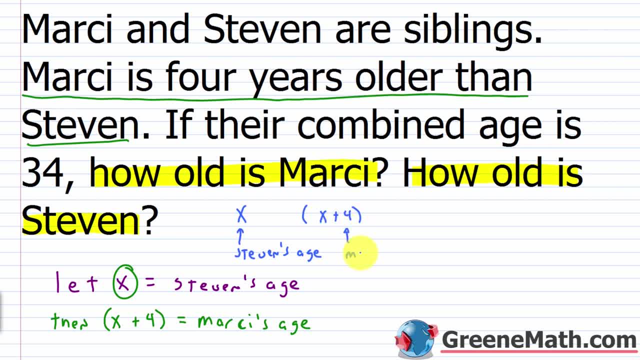 x plus four, that quantity, This is Marcy's age, And if I sum these two amounts together, it tells me here their combined age is, or equal to thirty-four. This is their combined age. So I've set up an equation and now I can just solve it. So let me. 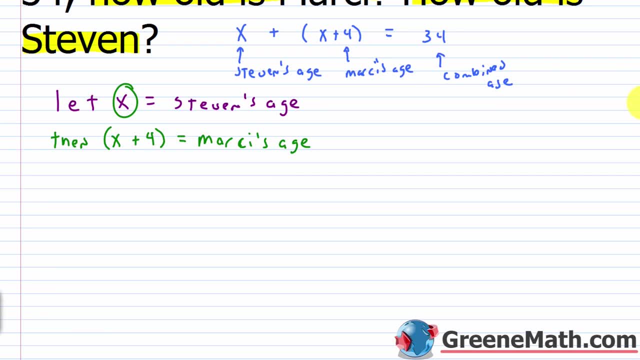 scroll down and get some room going. So if I have the equation x plus the quantity x plus four and this is equal to thirty-four- And I can just remove parentheses here- This would be two x plus four equals thirty-four. I would subtract four away from each side of the equation. 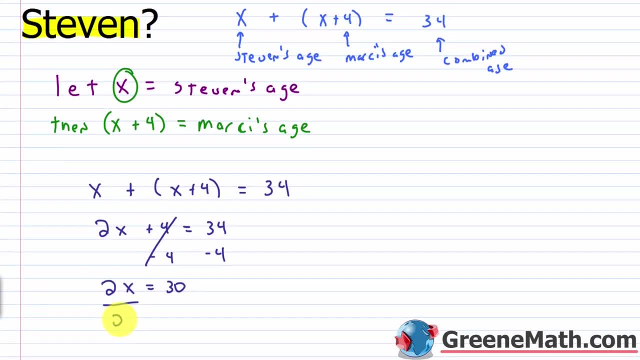 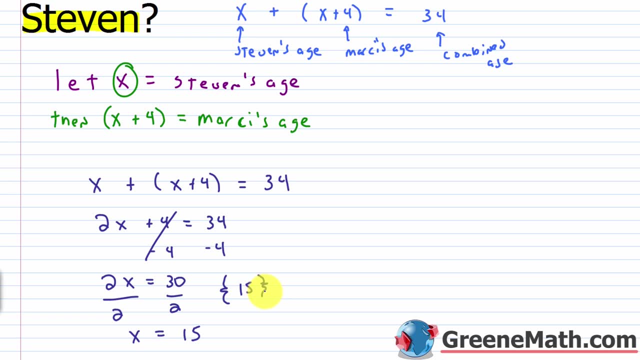 I would get two. x is equal to thirty. Divide both sides of the equation by two And I would get x is equal to fifteen. But when we're solving a word problem we don't just put x equals fifteen and then turn in the paper and say one hundred percent. 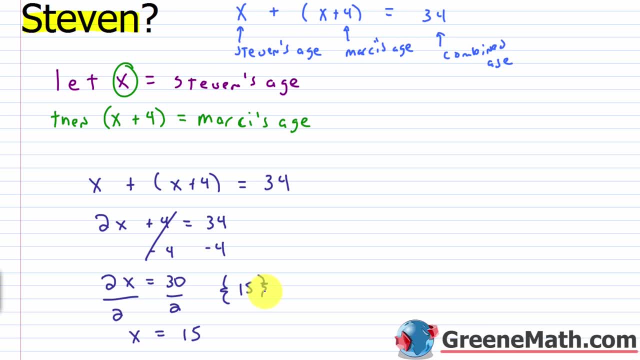 It doesn't work that way. We have to answer in terms of the problem. Now. we said that x was Steven's age, So that means that if x is fifteen, Steven is fifteen years old. So let me erase this And let me. 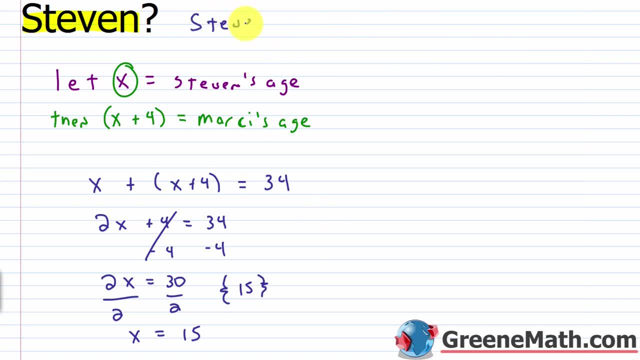 write that Steven is fifteen years old while Marcy is. and how old is Marcy? Well, Marcy's age is x plus four. If x is fifteen, I'm just plugging in a fifteen here. I'd have fifteen plus four or nineteen, So, while Marcy is nineteen. 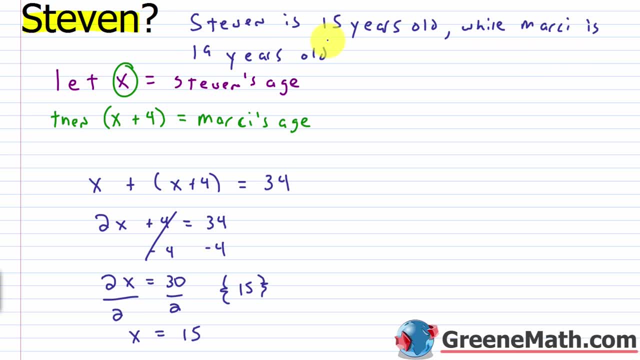 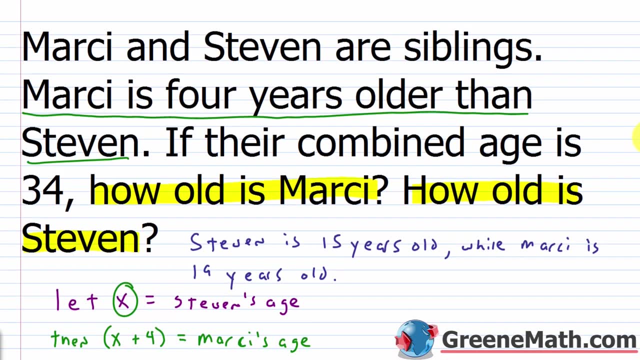 years old. Okay, so let's erase all of this And now let's check to make sure that this answer is reasonable. So if I go back up here, All you need to do is go back through the problem. Marcy and Steven are siblings. 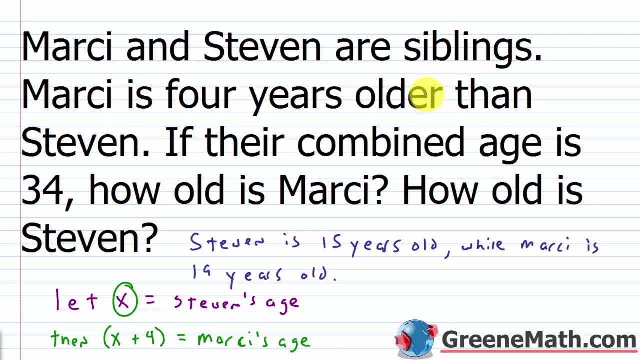 So that's not really relevant to us. Marcy is four years older than Steven. If I look at this, nineteen is four more than fifteen, So that checks out. If their combined age is thirty-four, So fifteen plus nineteen is thirty-four, So everything checks out. 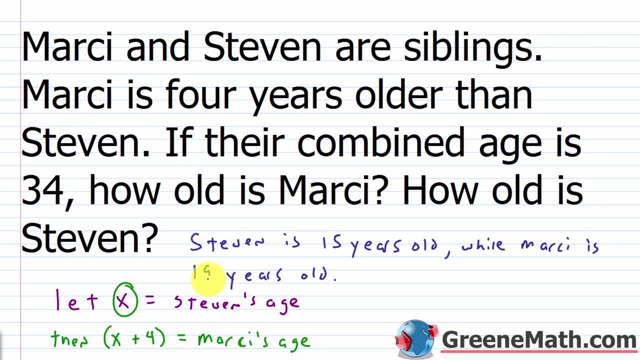 based on the information in the problem, We can say with a hundred percent accuracy that we know that Steven is fifteen years old, while Marcy is nineteen years old. Now one thing I want to show you real fast, Because a lot of you will say: well, what if I would have put x as Marcy's? 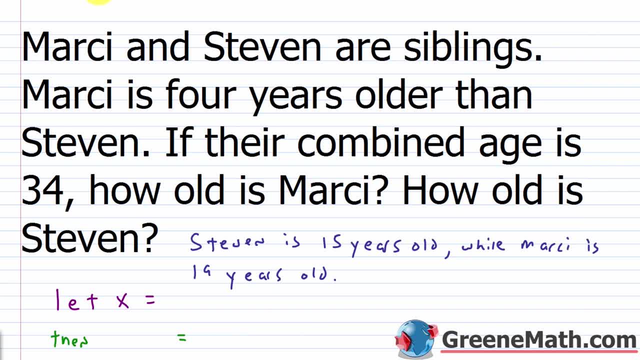 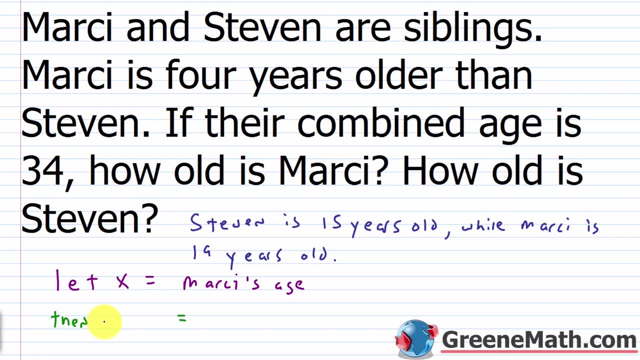 age to begin with. Okay, let's do that. Let's let x equal Marcy's age, And then we would have: what If Marcy is four years older than Steven? how do we properly represent Steven's age? Well, Marcy's age, which is represented with: 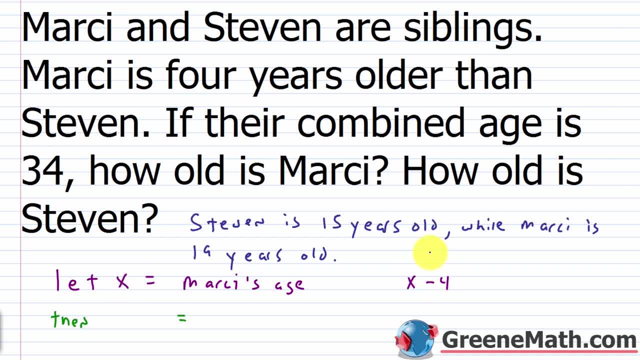 x, I'd have to subtract four away now to get Steven's age. So then x minus four, that quantity would be Steven's age. As an example, we already know that Marcy's age is nineteen. If I take four away from nineteen, I'd get 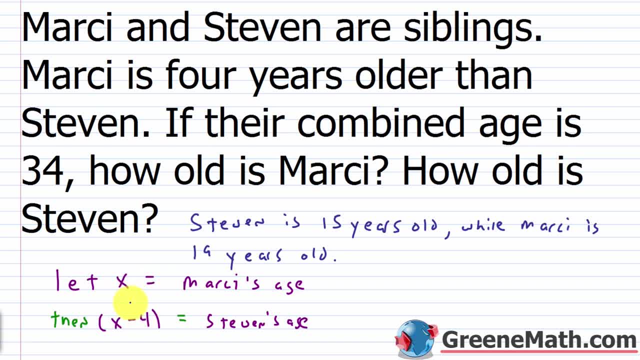 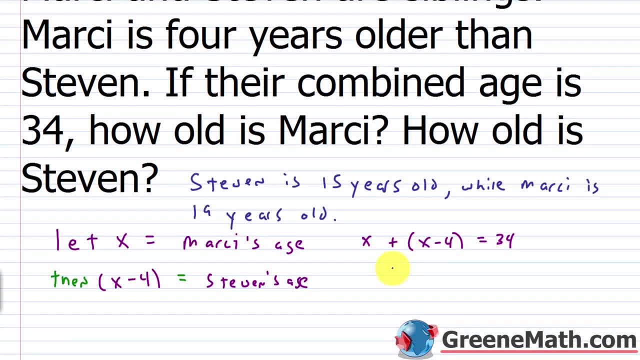 Steven's age, which is fifteen, And then I'd do the same thing to set up my equation. I'd have x plus the quantity x minus four, And this equals thirty-four. So I would get two x minus four equals thirty-four. Add four to each side of the equation. 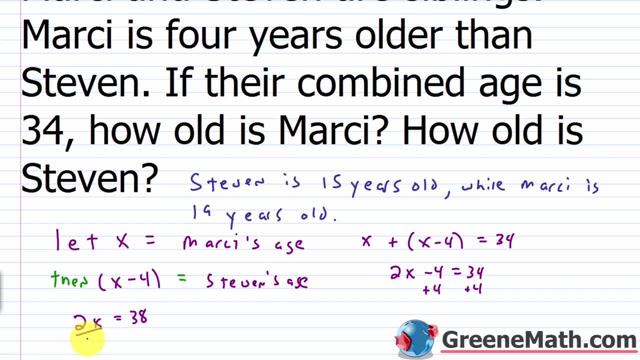 I'd have two. x is equal to thirty-eight. Divide both sides by two And I'd get x equals nineteen. You might say, aha, x equals fifteen before. Well, remember, x now is representing Marcy's age. We change that up And Marcy is nineteen. 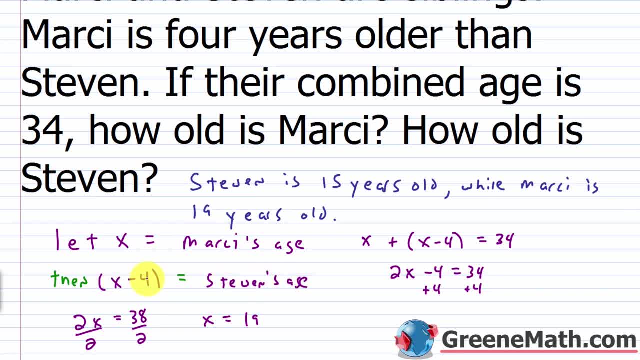 While Marcy is nineteen years old. To get Steven's age now, I subtract away four. Nineteen minus four would give me fifteen. So again, either way you set this up, you're going to get the correct answer. You just have to make sure. 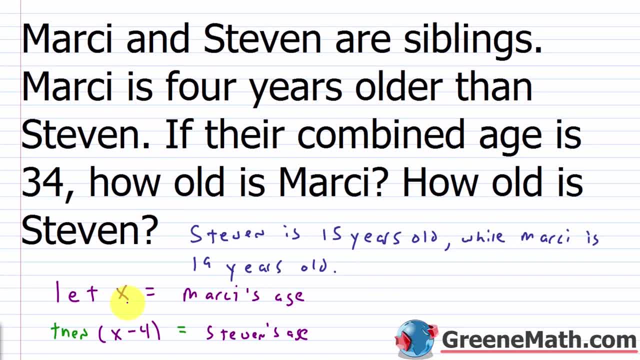 that you model everything correctly. Again, if you're letting x equals Marcy's age, then Steven's age has to be x minus four, Because Marcy is four years older than Steven. If you're letting x equals Steven's age, then Marcy's age has to be x plus four, Because, again, Marcy is four years older than Steven Alright. let's take a look at the next one. So during the sixteen game 2012 NFL regular season, the Broncos Chargers and Raiders combined to win a total of twenty-four games. The Chargers won three more games than the Raiders, but won six fewer games. 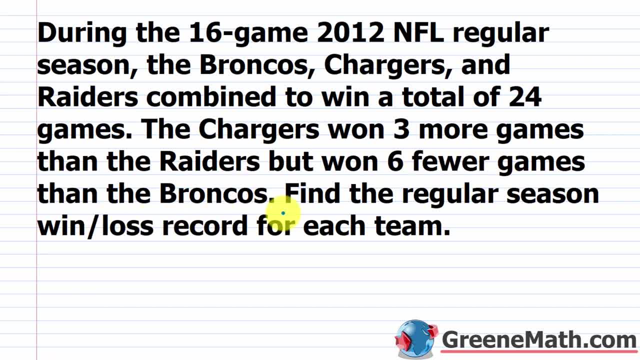 than the Broncos Find the regular season win-loss record for each team. Okay, so the idea here is that, at the end of the day, we want to find the regular season win-loss record for each team. So keep in mind that the regular season does not include. 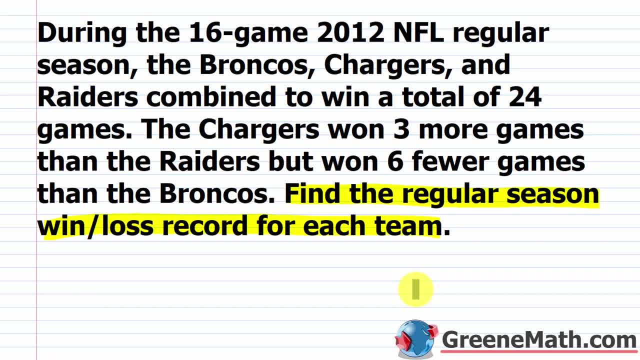 the preseason and it does not include the playoffs. Okay, so the records would be different if you included those extra games. It's also important to note that we're told that the 2012 NFL regular season consists of sixteen games, So we're going to use that in a little while. 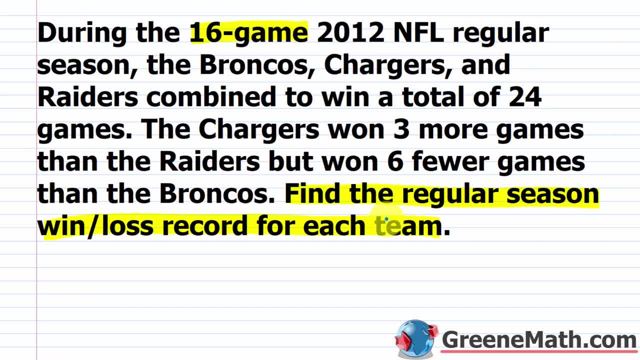 For right now, let's focus on the other information in the problem. What it tells us is that the Broncos Chargers and Raiders combined to win a total of twenty-four games. So that's very important. Let's highlight the twenty-four games. 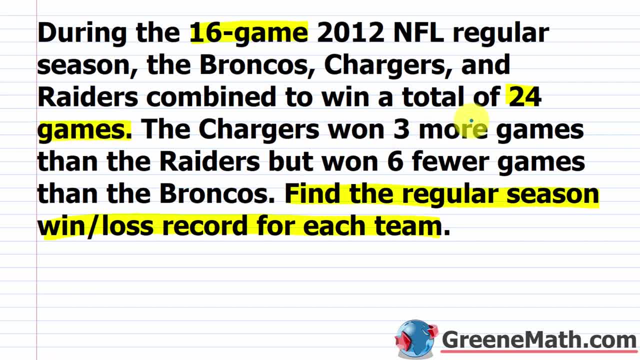 there. Then we're also told that the Chargers won three more games than the Raiders, but won six fewer games than the Broncos. So the idea here is that we could let X be equal to the number of games won by the Chargers. Let me start that off down here. Let's let X 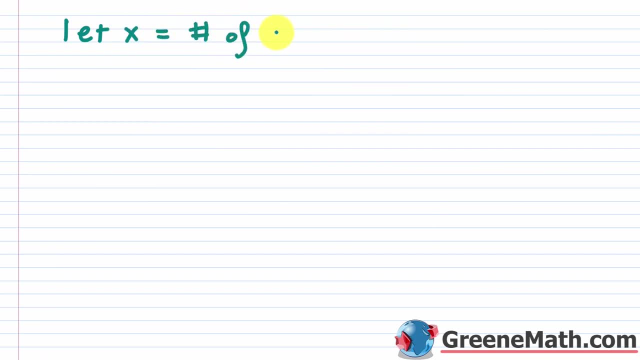 be equal to the number of games. we'll say one by- let me make this O a little bit better, and then we'll go the, and then we'll say Chargers. So that's the first part. Now the harder part, or the part that people struggle with, 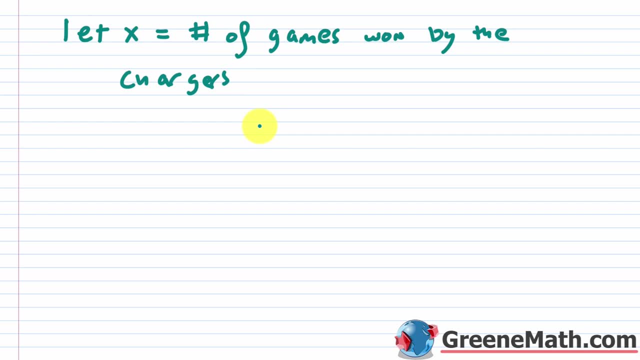 is then modeling how many games the Raiders won and how many games the Broncos won, based on this initial variable that we have. that's X, Again, the number of games won by the Chargers. So, coming back up here, if I just think about the Chargers won again, that's represented with: 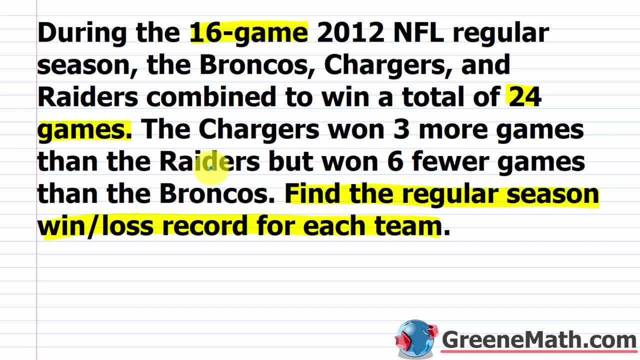 X- three more games than the Raiders. So that means the Raiders won three fewer games than the Chargers. So if the Chargers won X number of games, then the Raiders won X minus three number of games- again three fewer games. So we're just going to come back and say: 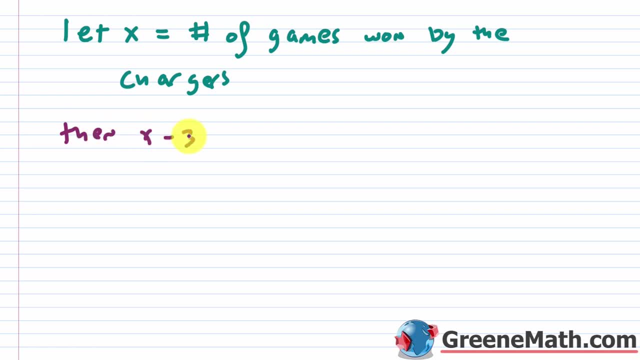 then X minus three- let me make this X a little bit better. this would be equal to the number of games, in this case, won by the, and we're dealing with the Raiders in this scenario. Okay, so the last team would be the. 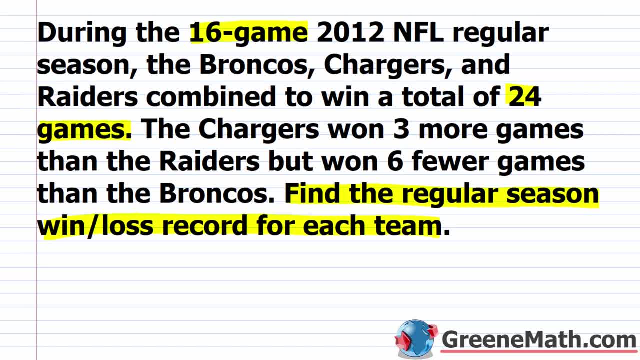 Broncos and they did better than the Chargers. It says here: the Chargers won three more games than the Raiders, but won six fewer games than the Broncos. So six fewer games than the Broncos. that means the Broncos won six more games than the Chargers. Again, if the Chargers won, 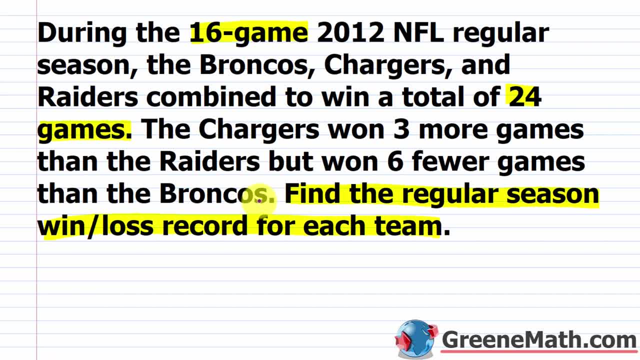 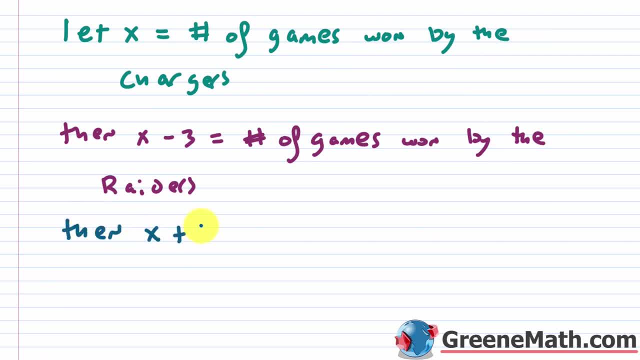 X number of games. now the Broncos won six more than that, so just X plus six number of games. So let's come back here and let's say: then we will say X plus six now would be equal to the number of games. 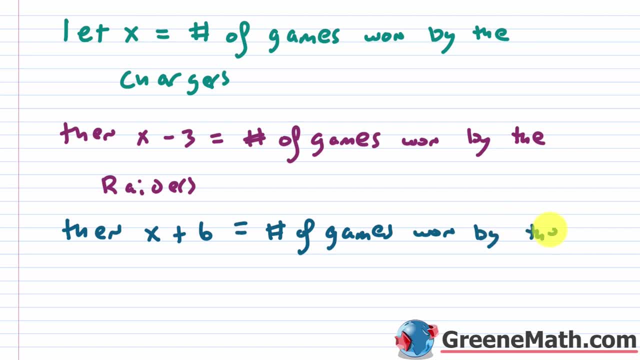 in this case won by the. we're dealing with the Broncos. Okay, so all we have to do to figure out what X is is set up a little equation. Again, if we go back- we highlighted this initially- it says the Broncos. 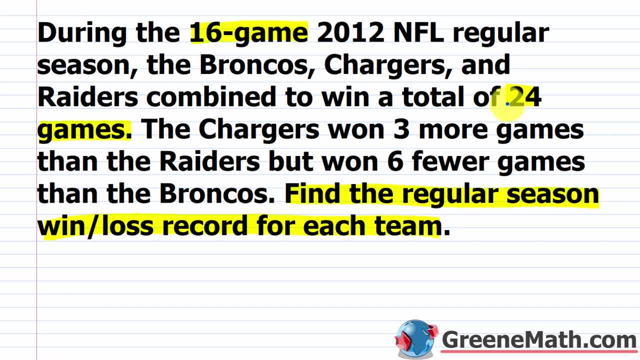 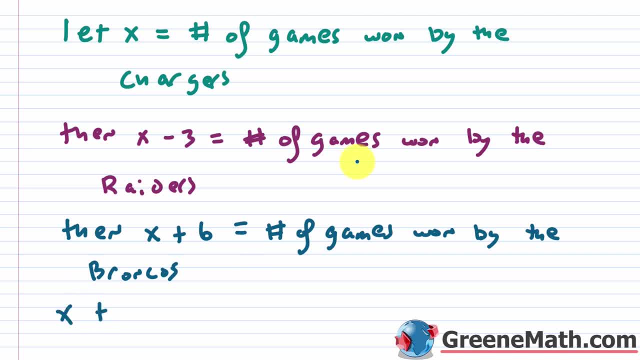 Chargers and Raiders combined to win a total of twenty-four games. So that's the key. That means, if I take the number of games won by the Chargers, which is going to be X, and I add that to the number of games won by the Raiders, 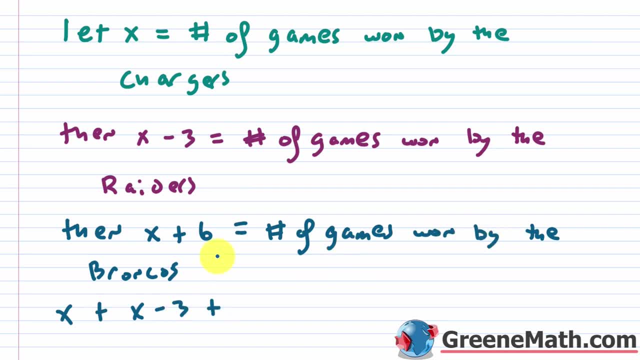 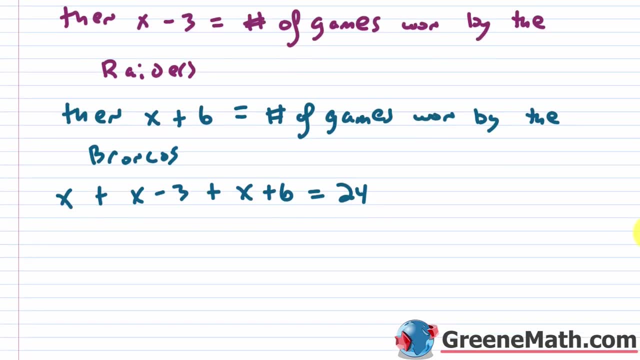 which is X minus three, and add that to the number of games won by the Broncos, which is X plus six, this sum should be twenty-four. Okay, let's solve this for X, and then we'll go back and figure out how many games the Chargers won, the Broncos won and the Raiders won, and then we'll figure out. 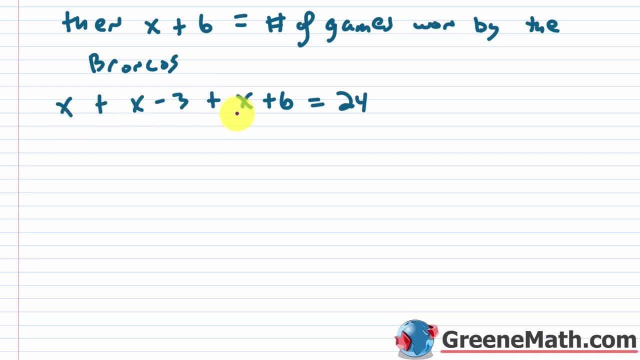 the win-loss record for each. So X plus X plus X would be three X. let's write that first. then negative three plus six would be plus three and this equals twenty-four. Let's go ahead and subtract three away from each side of the equation. let's cancel this away and we'll say: 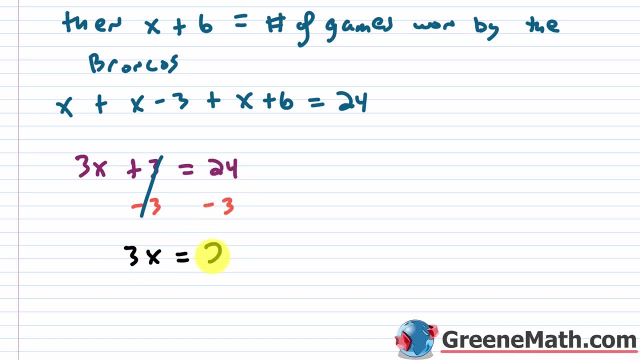 that three X is equal to twenty-four minus three is going to be twenty-one. As a final step here, let's divide both sides of the equation by three and we'll cancel this away and we'll say that X is equal to twenty-one. 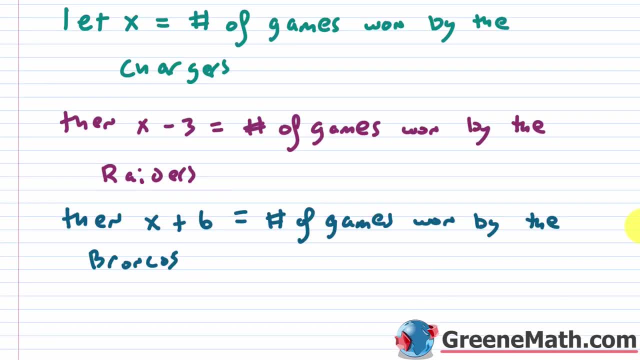 divided by three is seven, So X is going to be equal to seven. so, coming back here, we know that this would be seven for the Chargers. So let me just note this, that they won seven games. Then for the Raiders, it's seven minus three. 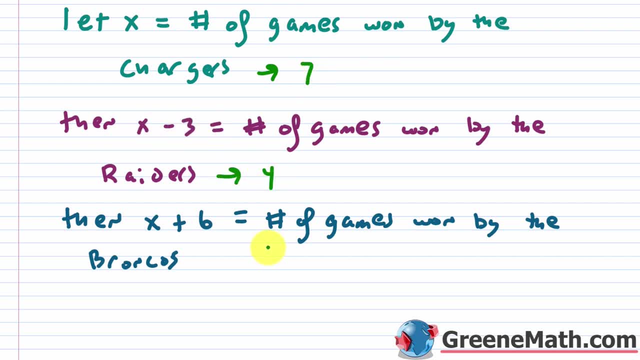 or four, so they won four games. Then for the Broncos, it's seven plus six, which is thirteen, so they won thirteen games. Alright, so I know how many games they won, but how do I figure out how many games they lost? Well, coming back here, remember. it says specifically the sixteen. 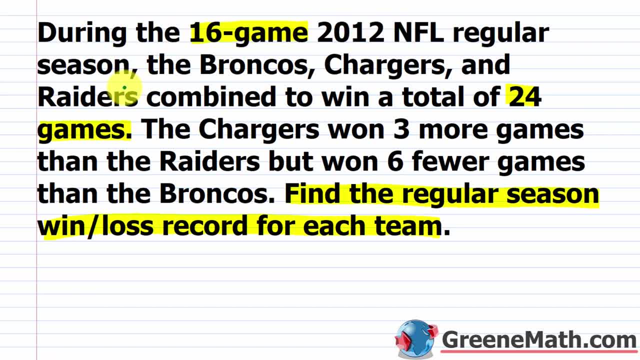 game: 2012 NFL regular season. So if they played a total of sixteen games, all I have to do is take that sixteen, subtract away the number of games they won and that'll give me the number of games they lost. So the Chargers again, they won seven games. So that means 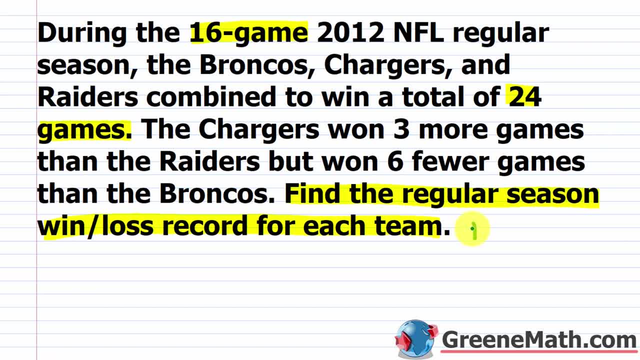 sixteen minus seven is nine. they lost nine games. So I'll just say the Chargers. the Chargers won seven games and we'll say they lost nine games. And again, if you want to make this a little bit shorter, you could just say their record was: 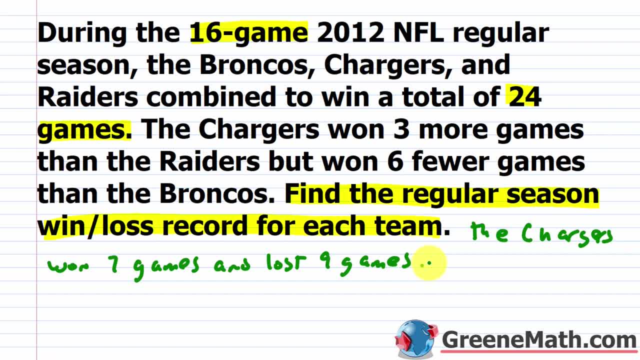 seven and nine. Most people know what that means. We can also say for the Raiders: they won four games, so sixteen minus four would be twelve, so their record would be four and twelve. We'll say maybe a comma here, while. 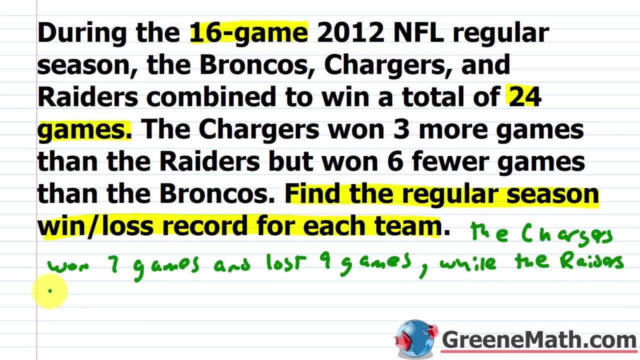 the Raiders will say won. in this case it would be four games, and they lost in this case twelve games. And then we'll say: and the Broncos, which would be the last team here, we'll say they won again, it was. 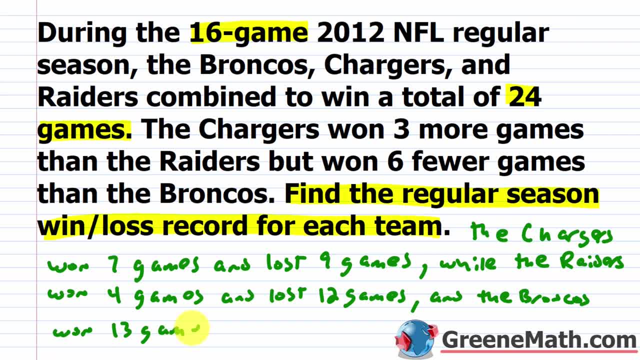 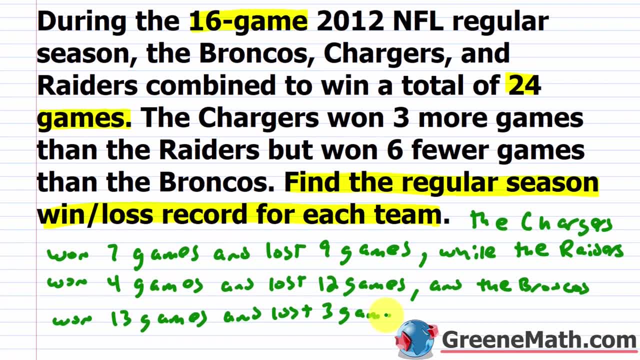 thirteen games. so we'll say thirteen games, and then sixteen minus thirteen would be three. so we'll say: and they lost three games, And that's pretty much it. I mean, you don't need this long of a sentence. In most cases something more simple would do. 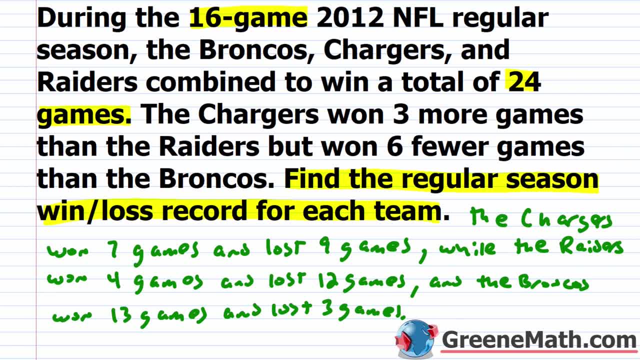 But just to be thorough, I wrote something like that And just to check things again, each team had to play sixteen games in the NFL regular season. So we have seven plus nine, that's sixteen. so that works. We have four plus twelve. 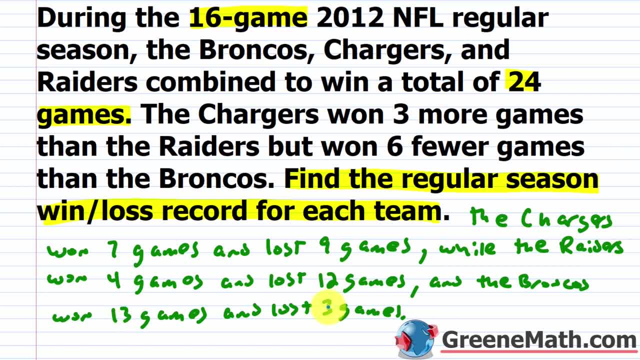 that's sixteen, so that works. And then thirteen plus three, that's sixteen, so that works. Then, additionally, you want to check that the sum of the wins would be twenty-four. So this part right here- So you have seven plus four- is eleven, and then 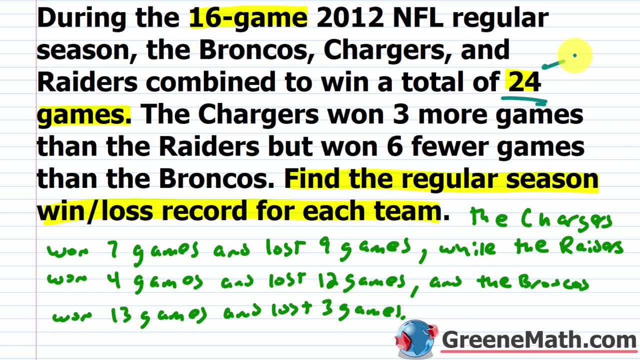 eleven plus thirteen, that is going to give you twenty-four. so that checks out. Then, additionally, you want to check this. So the Chargers won three more games than the Raiders. The Chargers won seven games. the Raiders won four games. so that checks. 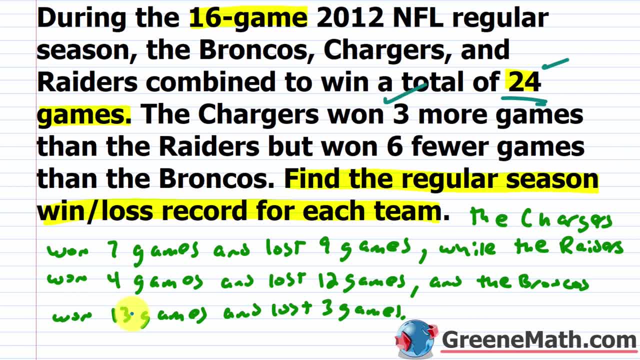 out. It also says six fewer games than the Broncos. The Broncos won thirteen games, the Chargers won seven games. so that checks out. So our solution checks out: The Chargers won seven games and lost nine, while the Raiders won four games and lost twelve. And then, lastly, the Broncos won thirteen games. 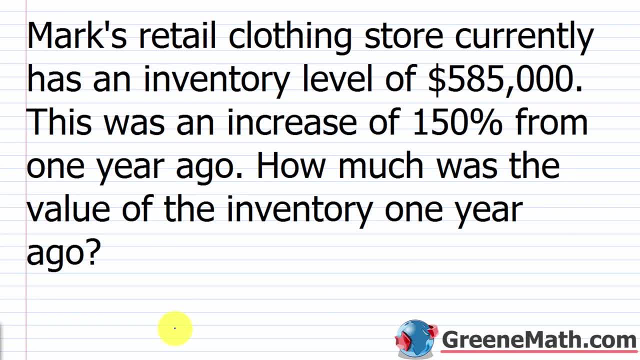 and lost three. So the next type of problem we're going to look at is a percent problem. These problems generally deal with a percent increase or a four percent decrease and we're going to be expected to find the original amount. So Mark's Retail Clothing Store currently has an inventory level of 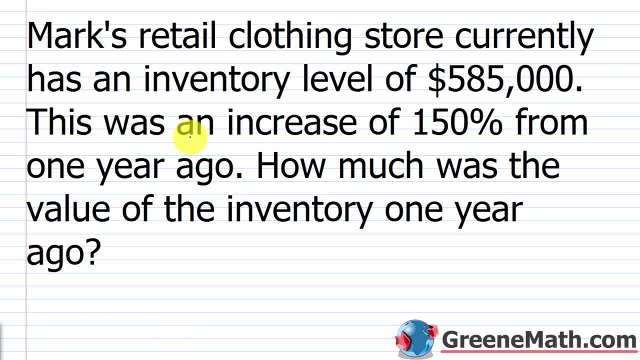 five hundred eighty-five thousand dollars. This was an increase of a hundred fifty percent from one year ago. How much was the value of the inventory one year ago? So this is what we're trying to find here. How much was the value of the inventory? 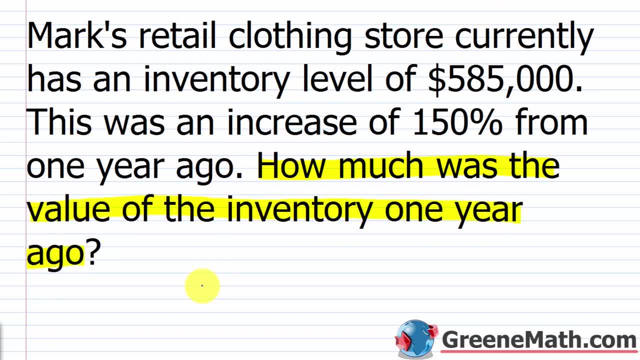 one year ago. So we can set a variable like x be equal to the value of the inventory one year ago. So how would I go about setting up an equation once I've determined that x is going to be the value of the inventory one year ago? Well, I've got to look at the 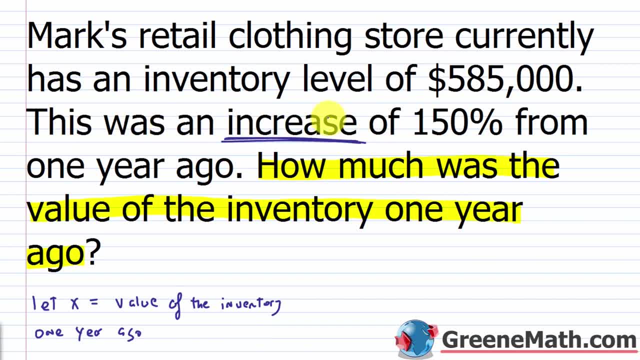 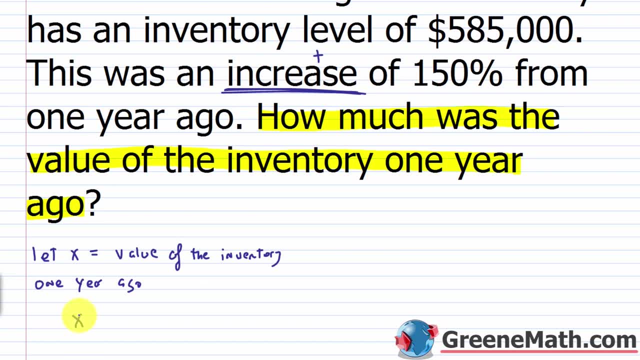 key words here. It says this was an increase. Increase means an addition, right? So if I started out with x, which is the value of the inventory one year ago, and I had an increase, or I added this amount, right here. 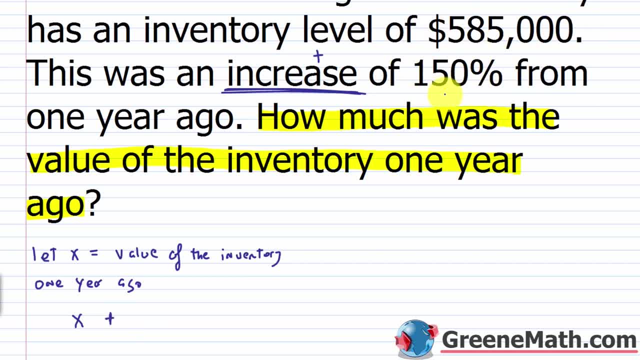 I know I would end up at this amount, So x plus the increased amount. and how would we get that? Well, it increased by a hundred fifty percent. So I would take the original value and I would multiply it by a hundred fifty percent. So in decimal form, a hundred fifty percent is. 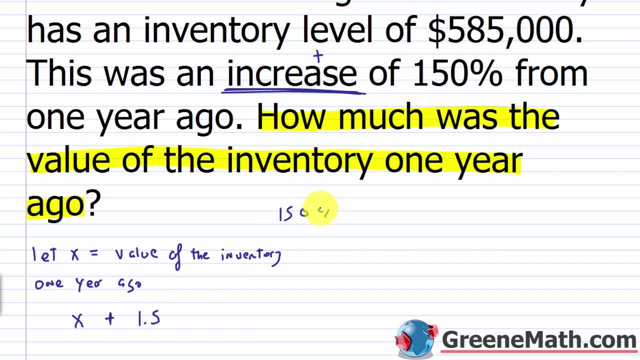 one point five. Alright, a hundred fifty percent is equal. to move this two places to the left, you get one point five. delete the percentage symbol. So this is one point five, and then times x. Let me label this real quick, so it's crystal. 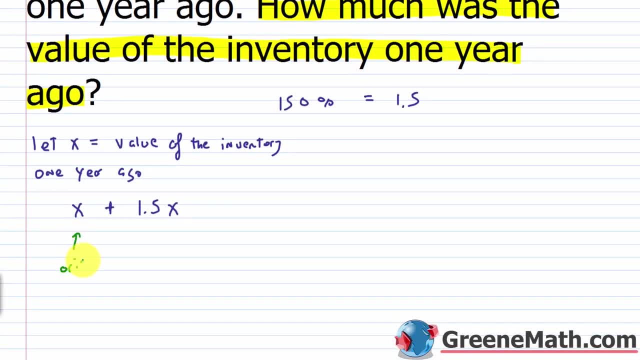 clear what's going on. This is the original and this right here is the increase, Because it's a hundred fifty percent of the original value. So one point five times x. again, x is the original. So if I do this, x plus one point five x. 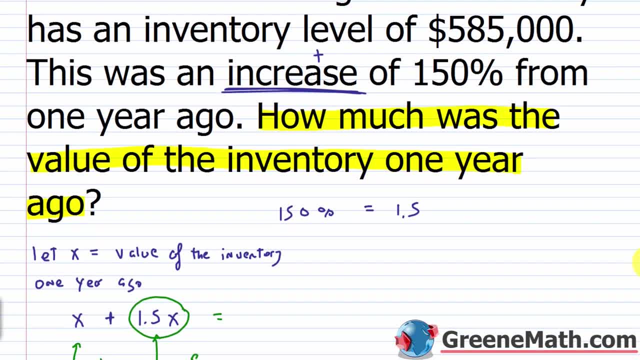 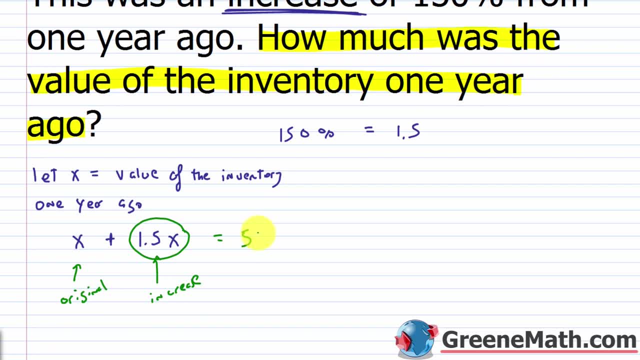 I know that, in terms of the problem, it tells me I should be sitting at five hundred eighty-five thousand dollars. So these two amounts will sum to five hundred eighty-five thousand, and then all I need to do is crank out my equation. 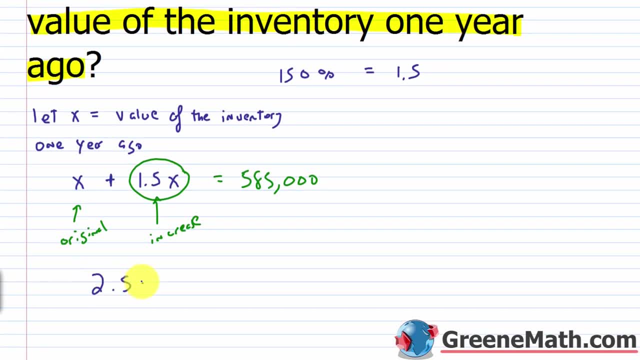 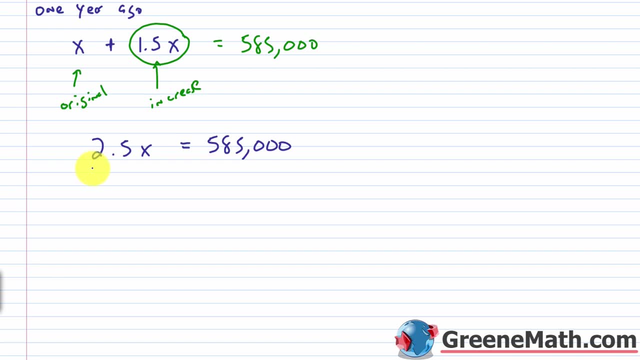 x plus one point five x is two point five x, and this equals five hundred eighty-five thousand. We would divide both sides of the equation by two point five and I would get that x is equal to two hundred thirty-four thousand. And again, that doesn't mean, I just stop. 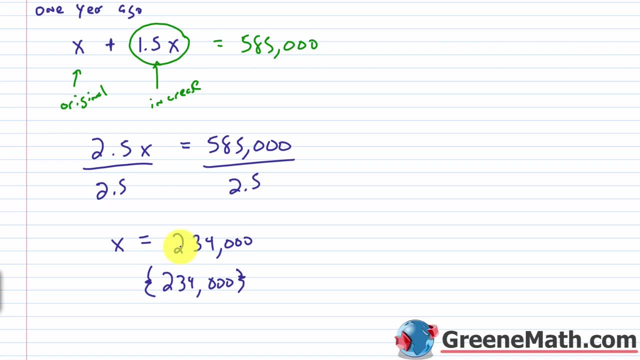 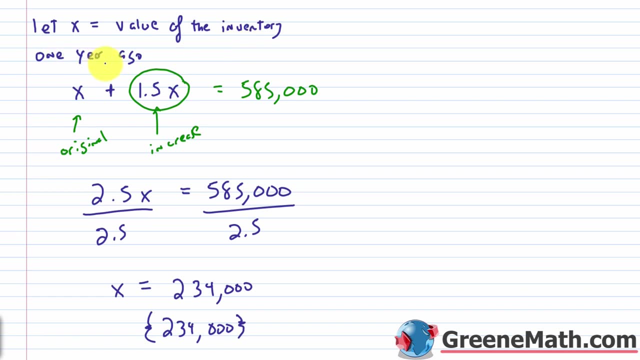 once I've written my answer down and I hand in my test and I say, hey, this is the right answer. I've got to translate that. Remember, x is the value of the inventory one year ago. So let me erase some stuff. 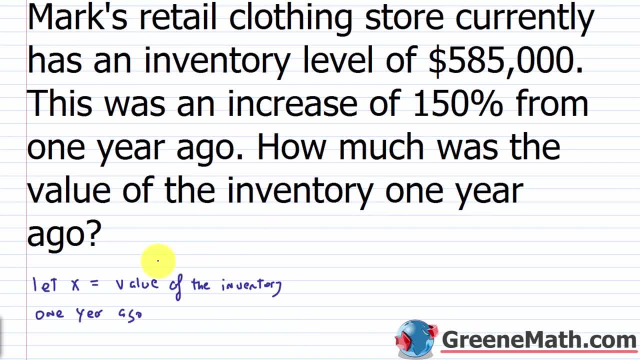 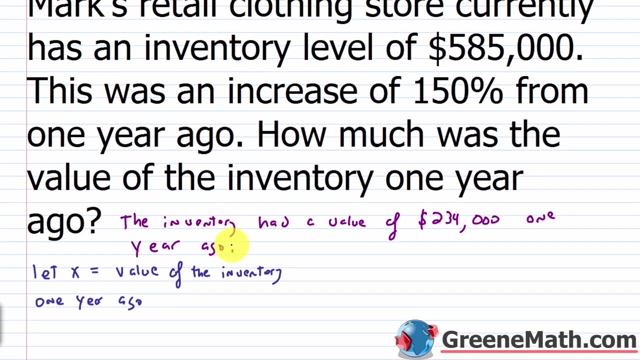 so I can fit this on a screen And what we're going to say is that the inventory had a value of two hundred thirty-four thousand dollars one year ago. Alright, and we can check that quite easily If we take two hundred thirty-four thousand. 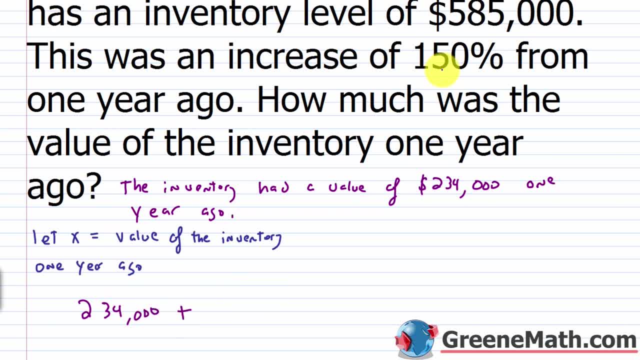 and we add to it the increase of a hundred fifty percent again, that's two hundred thirty-four thousand times one point five, that would be three hundred fifty-one thousand. If we sum these two amounts together, we do get five hundred eighty-five thousand. 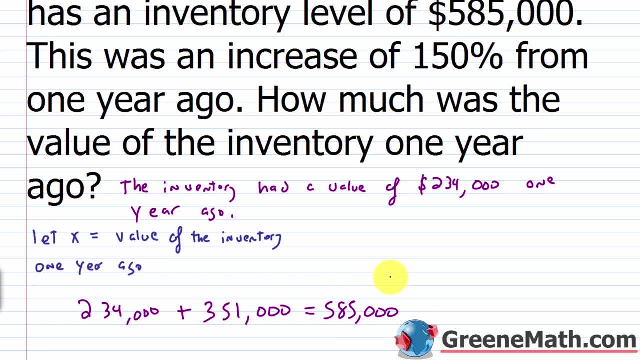 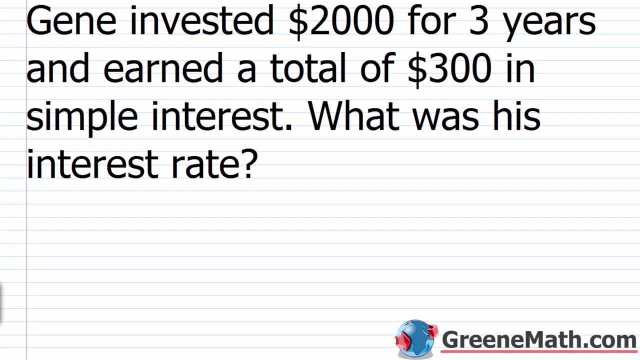 So that is consistent with what we have in the problem. so we can say here: our answer is correct. The inventory had a value of two hundred thirty-four thousand dollars one year ago. Alright, lastly, we're going to look at a simple interest problem, and we looked at this in a previous video where we 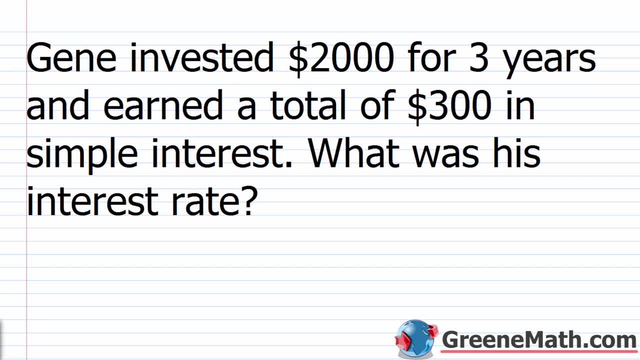 talked about formulas. So Gene invested two thousand dollars for three years and earned a total of three hundred dollars in simple interest. What was his interest rate? Now, when you get some of these problems, there's a formula you're going to use and 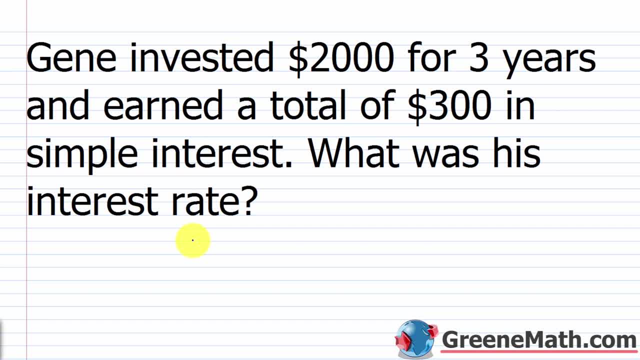 like with the motion word problems or with simple interest. you're going to see these enough to where you're going to have it memorized. So for this one you have, I is equal to P times R times T, where this is the amount of simple interest earned. 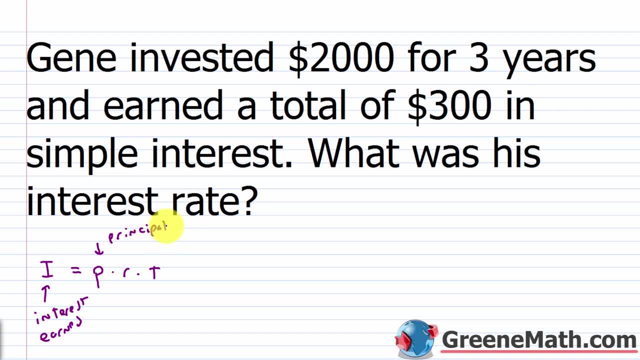 This is your principal, This is your rate And this is your time. Now this is asking us specifically: what was his interest rate? So in this particular case, I want to solve for R, because that's what I want to find. So 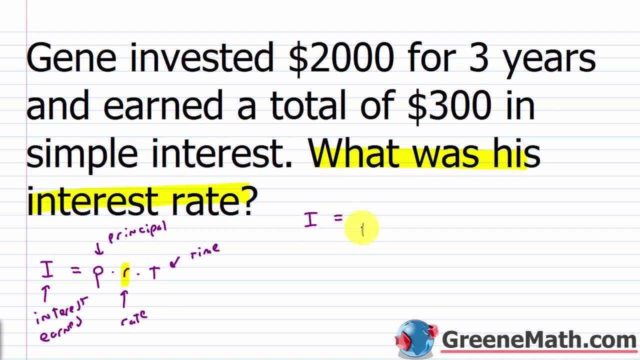 what I want to do here is divide both sides of this formula by Pt so I can isolate R. So I would have R is equal to I over Pt. Now, once I have this, let me just erase all this so I can kind of tighten everything up here. 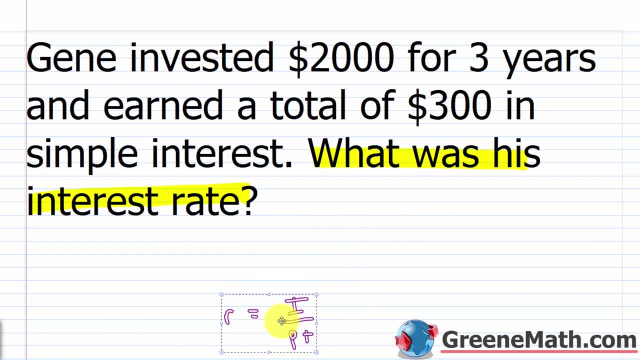 Once I have this, I'm pretty much good to go on this type of problem, Because I need to just plug in the amounts given. It tells me that Gene invested two thousand dollars, So that's my principal. Two thousand For three years. So my time is. 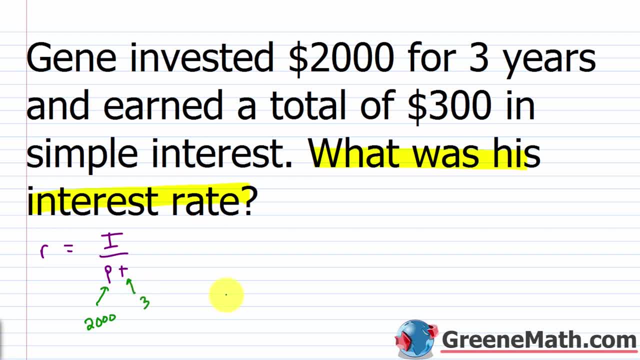 three, And it told me that he earned a total of three hundred dollars. So I would have three hundred, Which is the amount of simple interest earned is three hundred. So now I just have to crank this out and I have an answer. So what I'd end up with is: 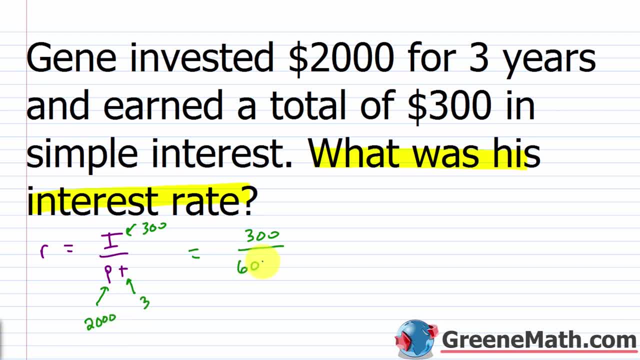 three hundred over two thousand times three. We know that's six thousand And without even using a calculator I can cancel these zeros with these zeros And I get three over sixty. Now I know sixty is divisible by three, It's twenty. So this is one over twenty, And 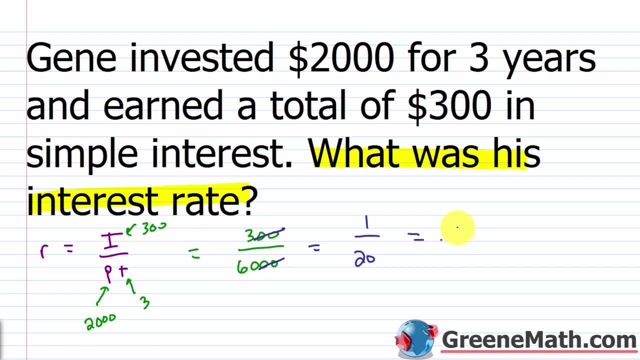 some of you can do that in your head. Some of you need a calculator But it ends up being point zero five, Point zero five, Or as a percentage. I move this two places to the right, I'd have five percent, So his. 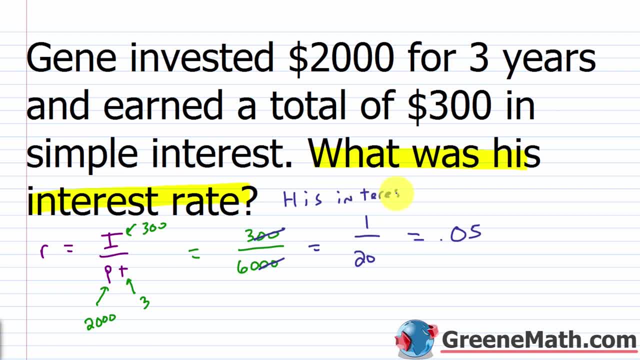 interest rate was five percent. Now again to check this. let me just erase everything real quick. Let's go to the original formula. So I, or the amount of simple interest earned is equal to. we know that the principal is two thousand. 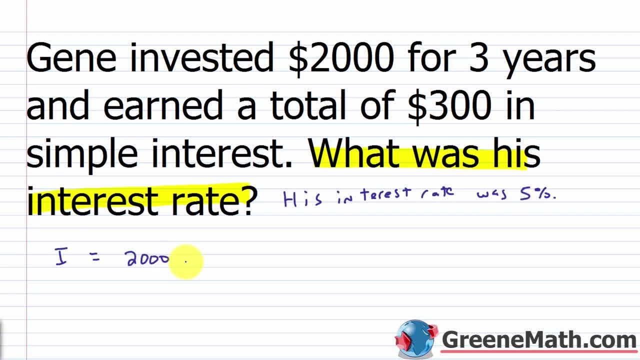 We know that the rate is five percent now, So let's put times point zero five. And we know that the time is three years, So let's put times three. So let's crank this out and see if it gives us three hundred dollars as an answer. So two thousand. 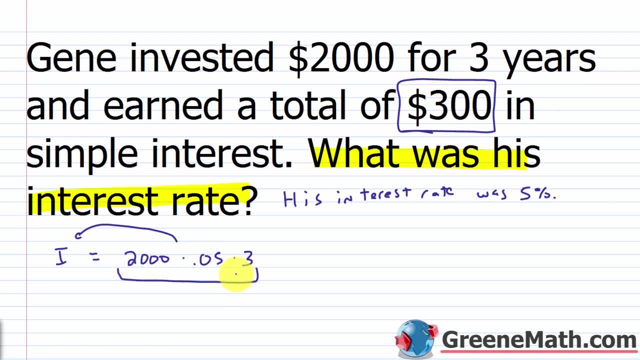 times three. we know that's six thousand. Six thousand times point zero five. yeah, we know that's three hundred. So this would be equal to three hundred, And so we can say our answer here is correct. His interest rate was five percent. Hello and welcome to Algebra 2, Lesson 9.. 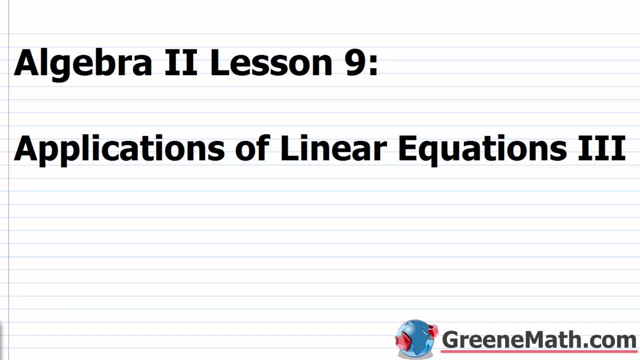 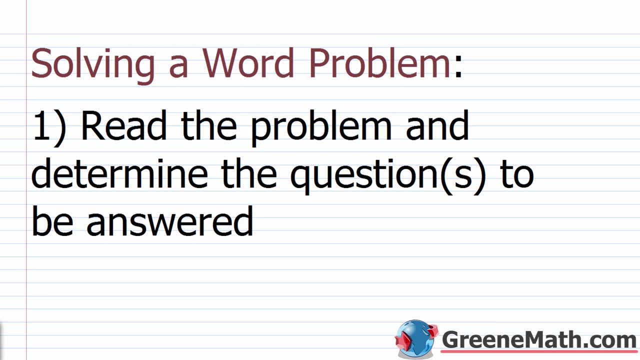 In this video we're going to continue to learn about applications of linear equations. So in this lesson I want to go over three additional types of problems that you're going to encounter. We're going to take a look at mixture problems. We're going to take a look at some denomination of money. 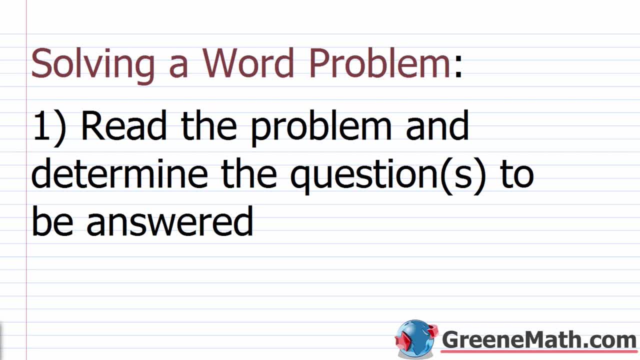 problems, And we're also going to take a look at some motion word problems. So before we get started, let's revisit our kind of guidelines for solving a word problem when you have to set up and solve a linear equation in one variable. So the first. 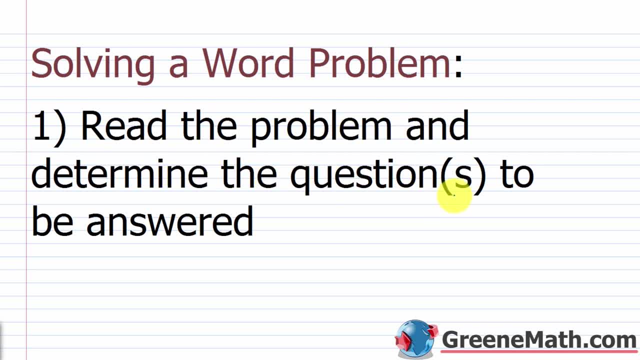 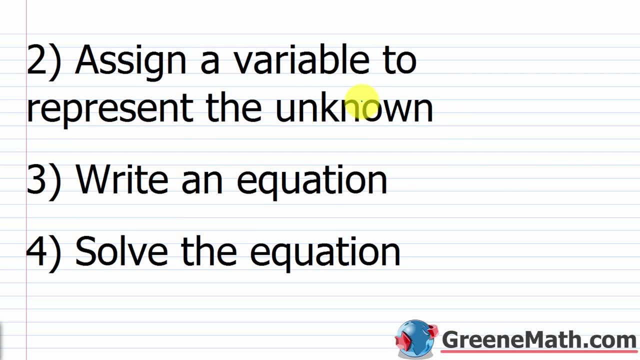 thing you want to do is read the problem and determine the question or questions to be answered. Then we want to assign a variable to represent the unknown, And if you have more than one unknown, you're going to represent other unknowns in terms of the value of the variable. 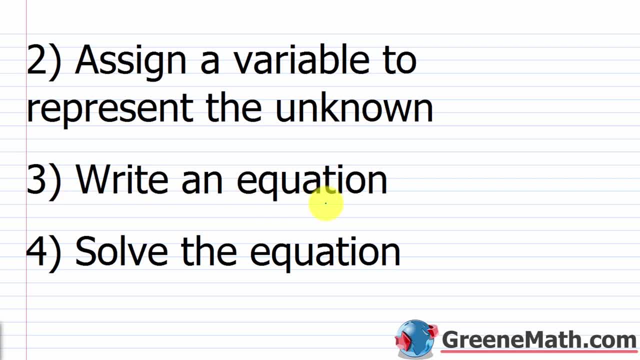 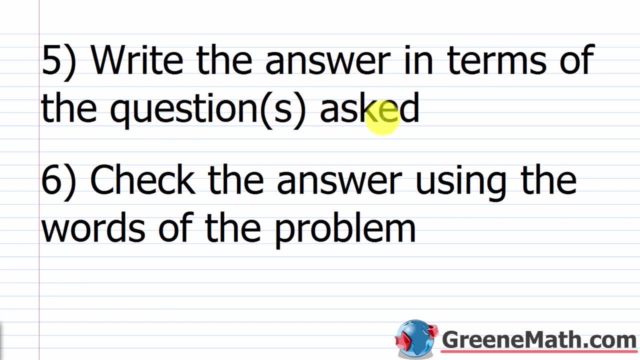 Then we want to write an equation, Then we're going to solve the equation, We're going to write the answer in terms of the question or questions being asked And then, lastly, we're going to check the answer using the words of the problem. And, again, the main thing with checking the answer. 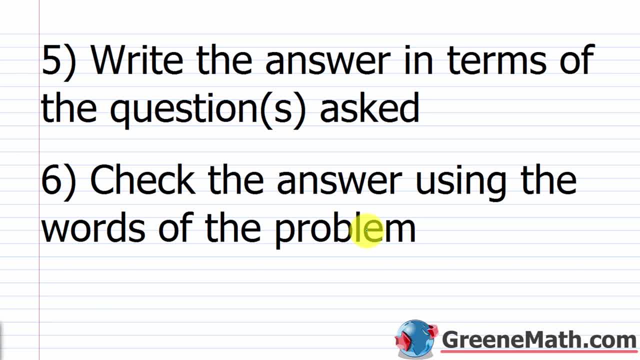 is to make sure that it's reasonable. I always use an example where I say: if you're asked to find the number of people on a bus or a train or a car and you get like negative 4.3, you know you did something wrong. You're not going to have. 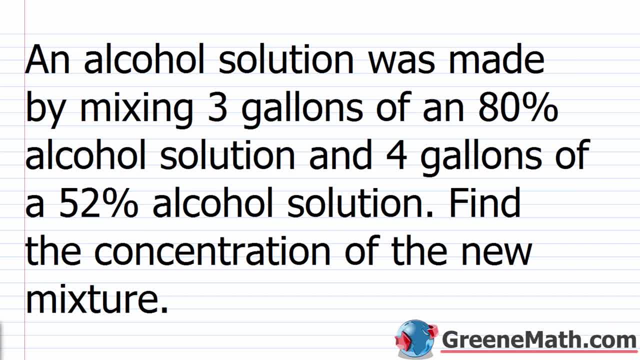 a negative amount of people on a bus. At this level, when we talk about linear equations in one variable, our mixture problems will involve basically rates of concentration. So let's read through this real quick. This is a nice little starter problem for us. It's going to teach us how to find the concentration. 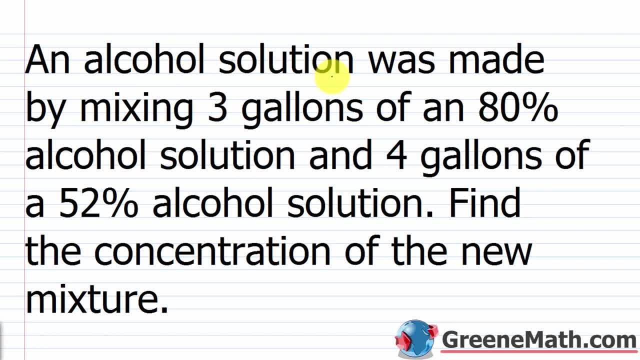 of a substance. So an alcohol solution was made by mixing 3 gallons of an 80% alcohol solution and 4 gallons of a 52% alcohol solution. Find the concentration of the new mixture. So how do we go about doing this? 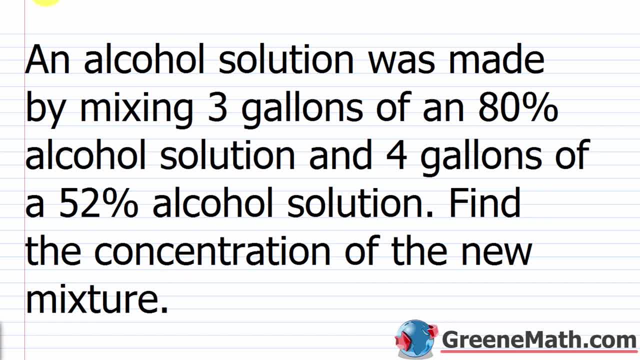 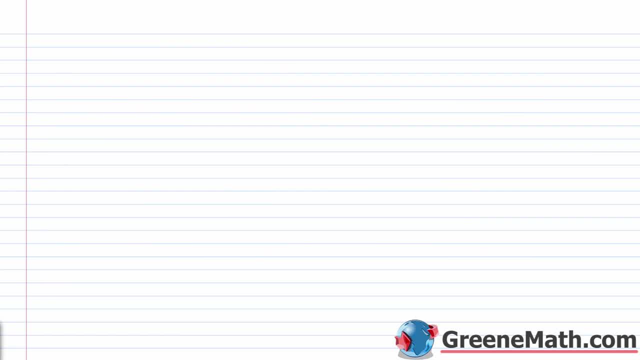 Well, what I want you to do is take a piece of paper and a pencil out, if you don't already have one, And I want you to write this down. Let me go to a different page. If you want the concentration of a substance, 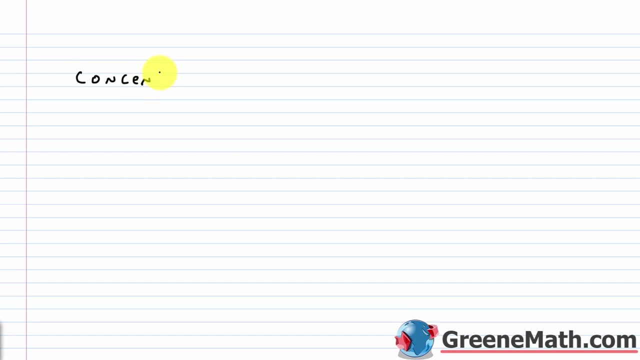 I'm going to write this down. So, concentration of the substance: This would be equal to: you need the pure amount of the substance And this is over or divided by the total amount of the mixture. So once you understand this right here, it's going to be really easy for you to do these mixture. 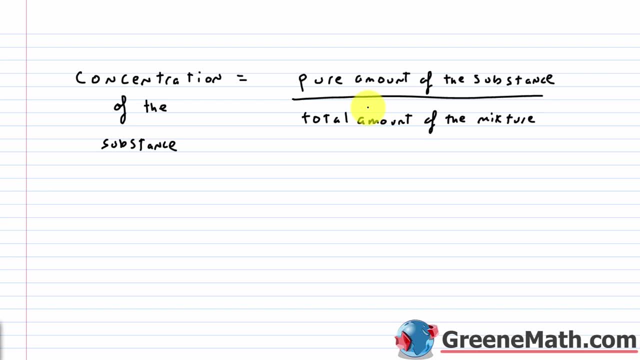 word problems. I can't tell you how many students I've tutored and they don't even understand this and they're trying to solve the problem. You have to know how to get the concentration of the substance before you can do anything. So let's go back up and we're going to fill in this information here. 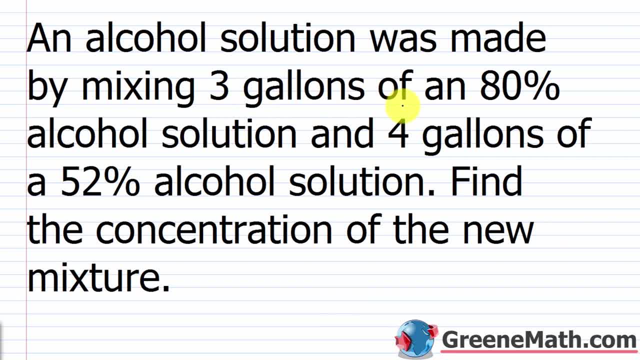 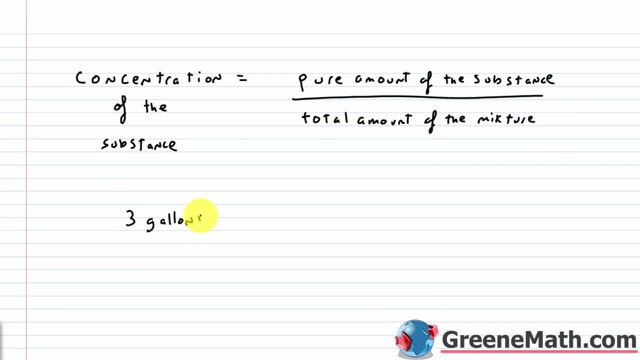 Now the information we're given is that there's 3 gallons of an 80% alcohol solution and 4 gallons of a 52% alcohol solution, So let's use this down here. So if I've got 3 gallons of again an 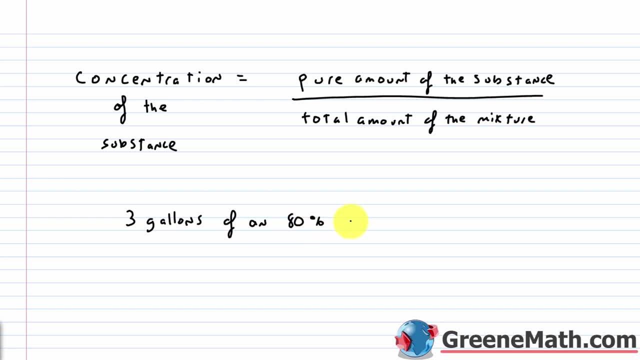 80% alcohol solution. I'm going to multiply it. by how much pure alcohol is that? Well, I basically just take 3 and I multiply it by 80% or .8 as a decimal. So 3 times .8 gives me 1.. Well, 3 times 8 is 24. 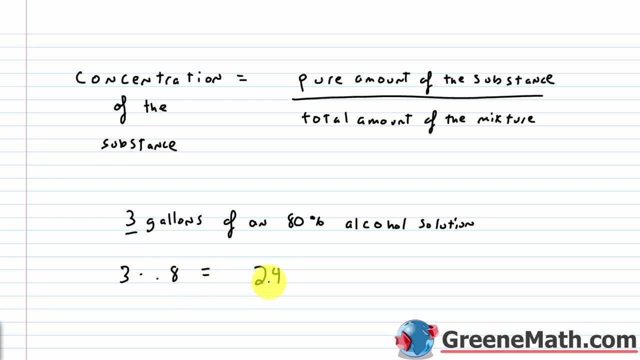 and I have one decimal place between the two factors. So this is 2.4.. And think about your units. there it would be gallons. So basically, 3 gallons of an 80% alcohol solution is 2.4 gallons of pure. 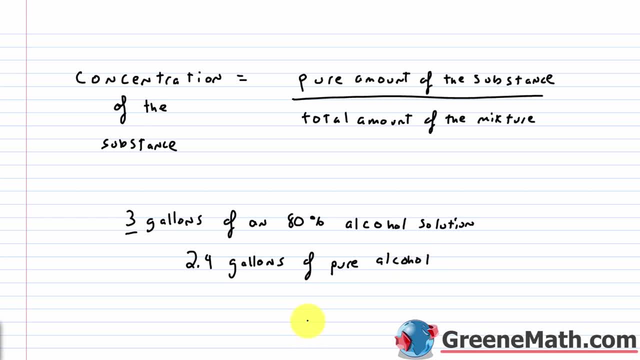 alcohol. So when we think about the pure amount of the substance again from this I'm going to have- let me just write it right here- I'll have 2.4 going in there. Let me erase this real quick And I'm going to put my fraction bar And then in here. 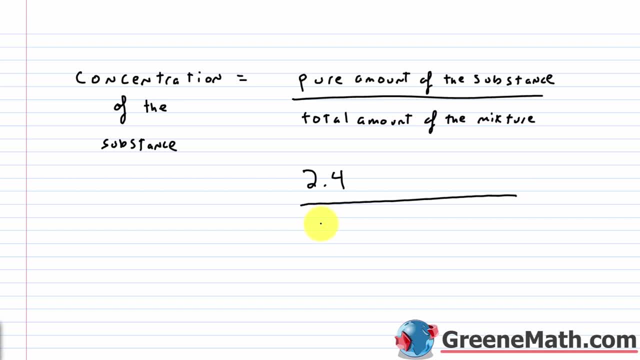 total amount of the mixture. I know this came from a 3 gallon mixture. Now I'm going to add to this and I'm going to add to this. Remember we had another part. We were mixing this with 4 gallons of a 52% alcohol solution. 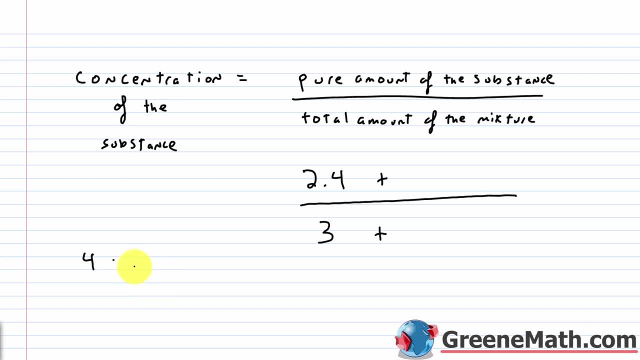 So 4 times 52% as a decimal is .52,. 4 times 52 is 208.. You've got 2 decimal places between the factors, So this is 2.08.. So again, this is how much in gallons that we have as a pure amount. 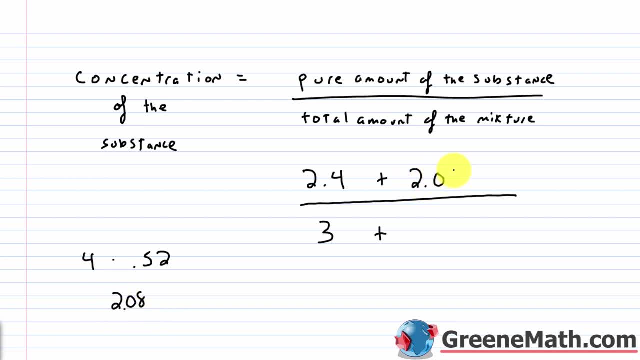 of alcohol. So this goes up here: 2.08.. And the total mixture is 4 gallons. So that goes here. So what do we have in the numerator? Again, we have the pure amount of alcohol from the first mixture. 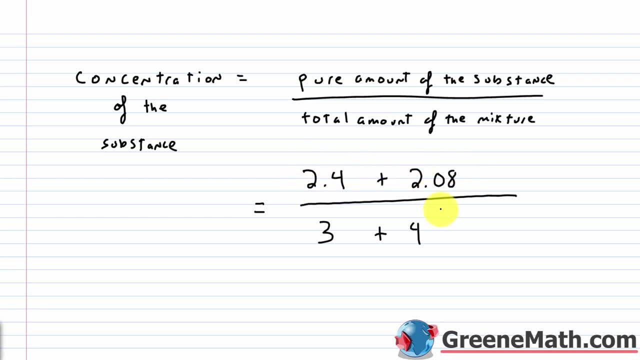 plus the pure amount of alcohol from the second mixture. So the numerator is the pure amount of the substance. In this case it's alcohol. So 2.4 plus 2.08 gives me 4.48.. And this is over The total amount. 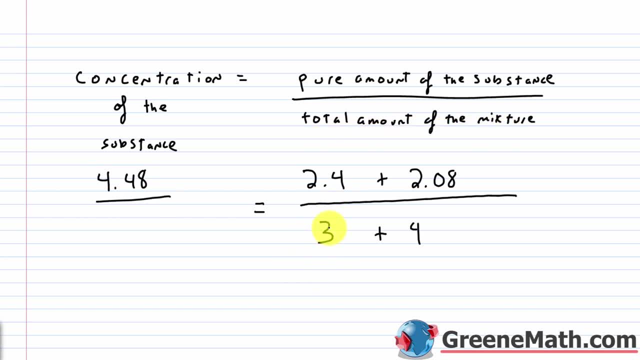 of the mixture. The first mixture was 3 gallons in total. The second mixture was 4 gallons in total. So 3 plus 4 would give me 7.. Now all we need to do is crank this out, So 4.48 divided by 7. 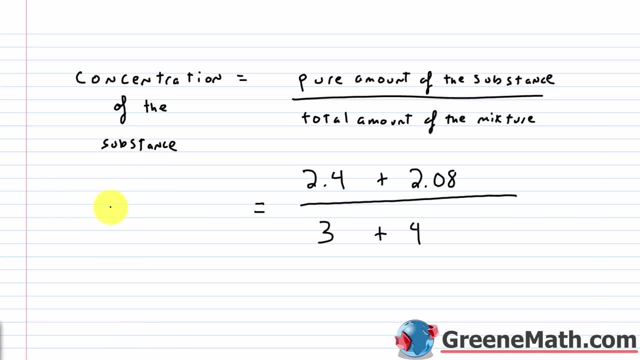 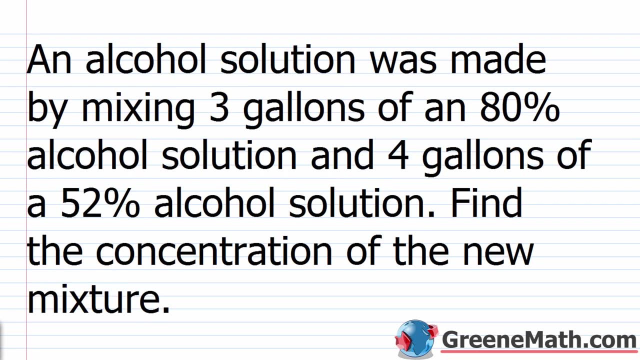 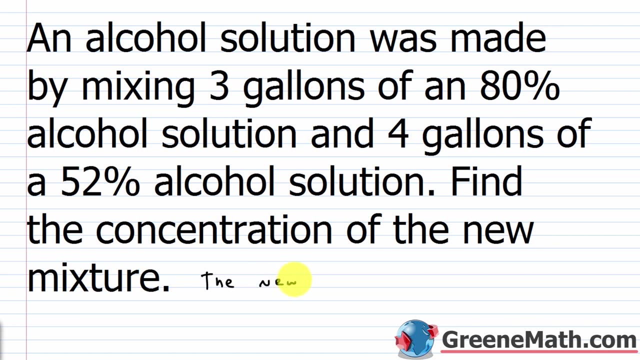 is .64.. So you can erase this and put .64.. And we know as a percentage that's 64%. So let's go ahead and answer this with a nice little sentence: Find the concentration of the new mixture. The new mixture is 64%. 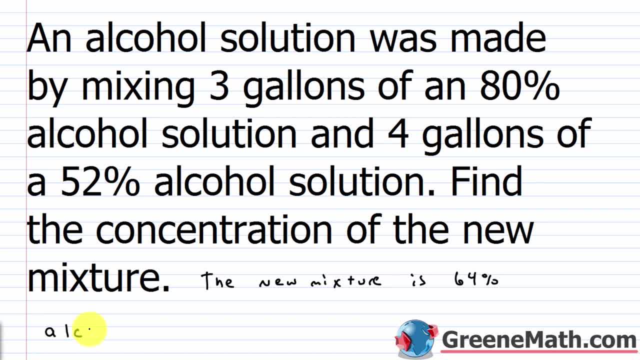 alcohol A-L-C-O-H-O-L, And it's really that simple. This is a very easy problem. I mean you just go through the kind of formula that I gave you, But make sure you have that written down, because a lot of times you're going to need to know how to find the concentration. 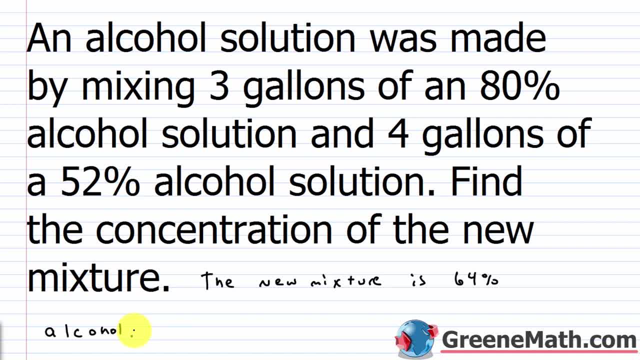 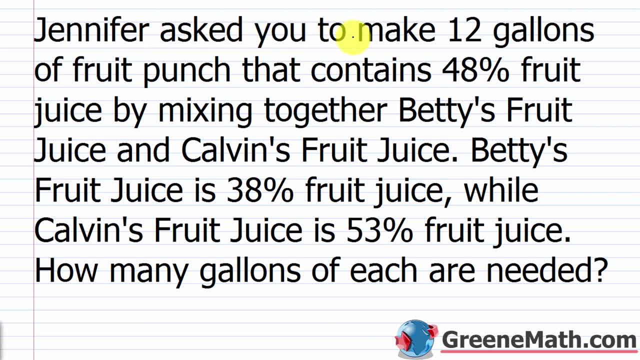 of a certain substance that comes from. you know mixing one or more items, Alright, so now let's take a look at one that's a little bit more challenging. So Jennifer asked you to make 12 gallons of fruit punch that contains 48% fruit juice. 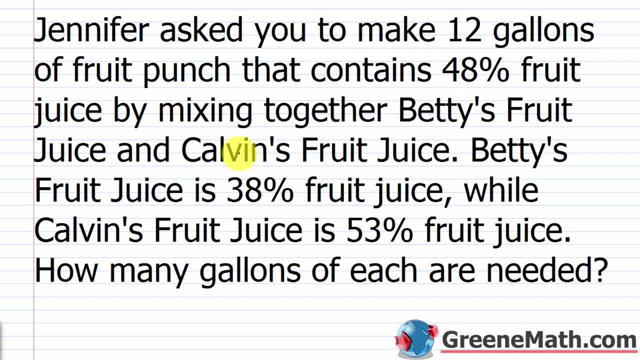 by mixing together Betty's fruit juice and Calvin's fruit juice. Now, Betty's fruit juice is 38% fruit juice, while Calvin's fruit juice is 53% fruit juice. How many gallons of each are needed? So a lot of times, with mixture problems, we get very, very. 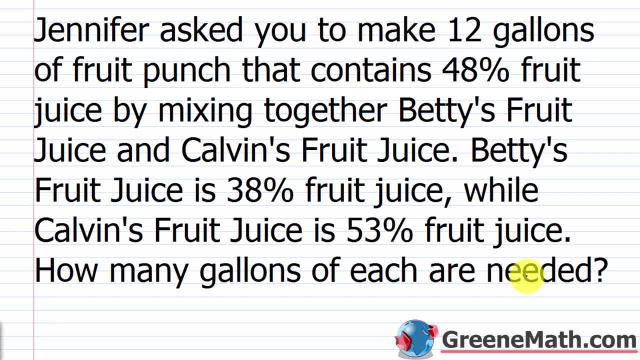 confused on what we need to do. I want you just to think about the fact that in the end, I want a 12 gallon mixture that is 48% fruit juice. So that's the goal. So let's write that down here. Our 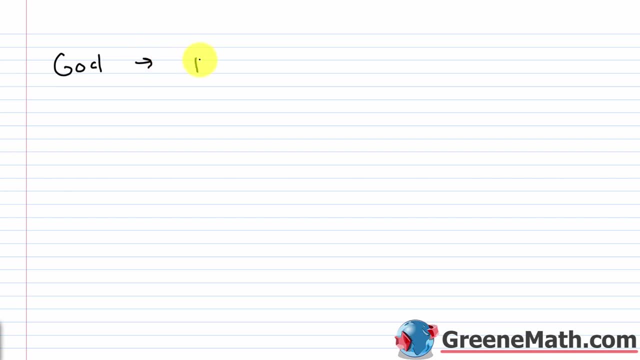 goal is 12 gallons, that is 48% fruit juice. So how are we going to get that? Well, we've got to use Betty's fruit juice and we've got to use Calvin's fruit juice. We don't know how much of each we're going to use, But we 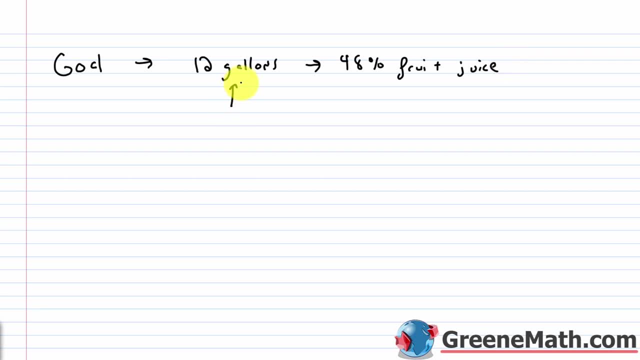 do know that we're going to take a total of 12 gallons for the mixture. So this is my total mixture in gallons. So if I let X be equal to the number of gallons of, let's say, Betty's fruit juice and we'll put used, then what can I say about? 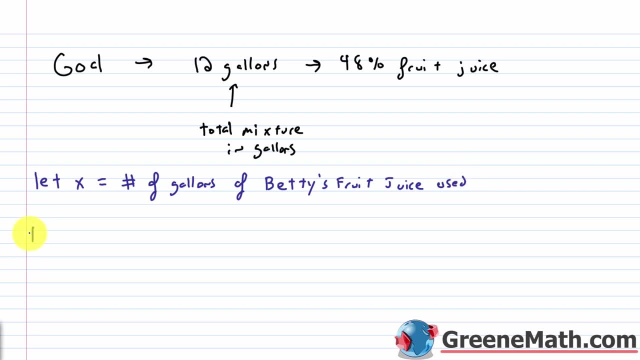 the amount we're going to use from Calvin's fruit juice. So then, well, if this is in terms of gallons, and it's the whole amount we're using- remember, the total mixture is 12 gallons, So whatever I use here can be subtracted away from 12.. In other words, if I had 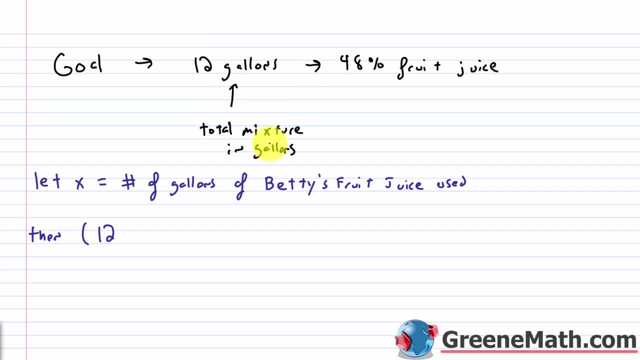 12, the total number of gallons from this mixture in the end, minus X the number of gallons we're using from Betty's fruit juice. well, that's got to give me the number of gallons of Calvin's fruit juice used, And of course you could have reversed that and said: 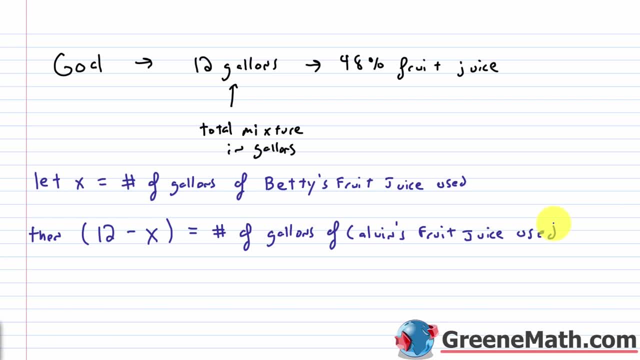 X is the number of gallons of Calvin's fruit juice used, And then 12 minus X would have been the number of gallons of Betty's fruit juice used. Doesn't matter, You'll get the same answer either way. Now how do we go about making? 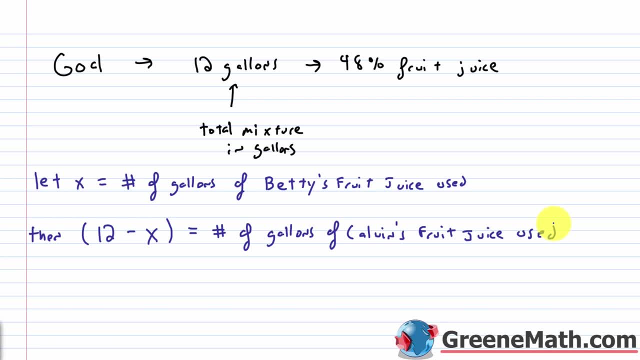 We've got our unknowns expressed with some variables. How do we make an equation? Well, the one thing is that we know that, in the end, the amount of pure fruit juice from Betty's fruit juice plus the amount of pure fruit juice from Calvin's fruit juice has 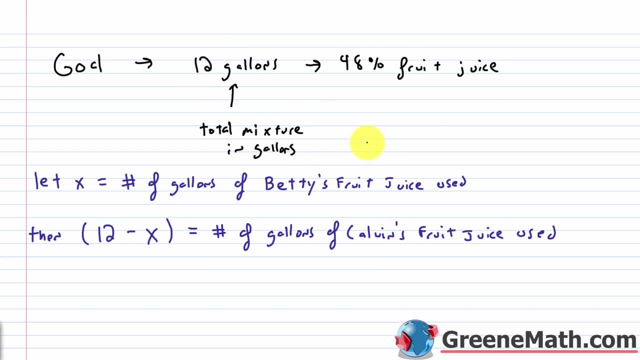 to equal the amount of pure fruit juice in the goal mixture. So in other words, we know that Betty's fruit juice is 38% fruit juice. So if I use 0.38, that's 38% as a decimal and I multiply it times x, this is the pure. 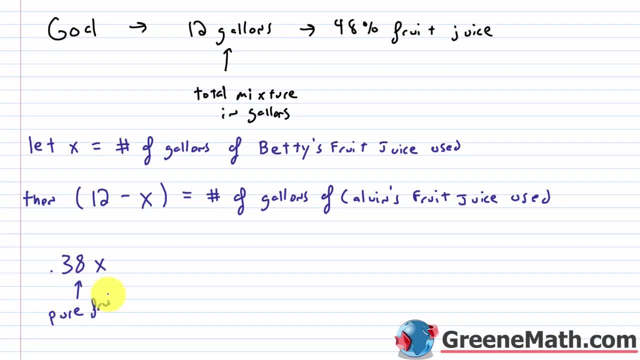 fruit juice And this is from Betty's. Okay. Okay, Now if I add this to- and I'm going to do the same thing for Calvin's fruit juice, So if I add this to his is 53% fruit juice. so 0.53 as a decimal times this quantity. 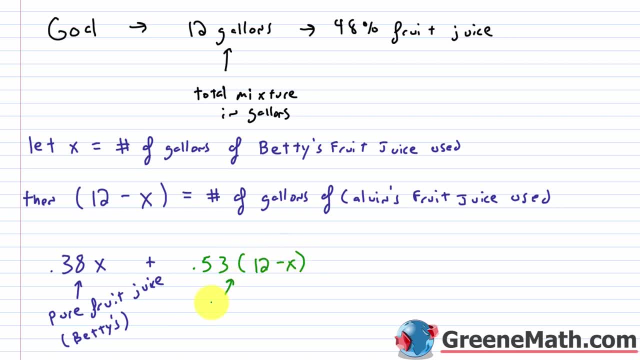 12 minus x. this is the pure fruit juice, And in this case it's from Calvin's. If I sum these two amounts together, it's got to be equal to the amount of pure fruit juice in the end mixture, So in other words, it would be 12 times 0.48.. 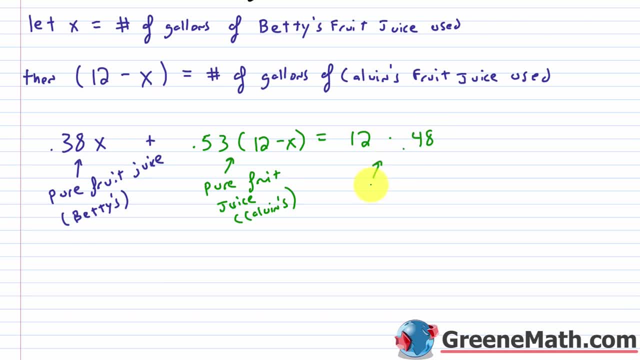 And this is the pure fruit juice in the final mixture. Okay, Okay, Okay, Okay, Okay. So this is the pure fruit juice in the end mixture, And what does that mean? It means that the final mixture comes from these two inputs. 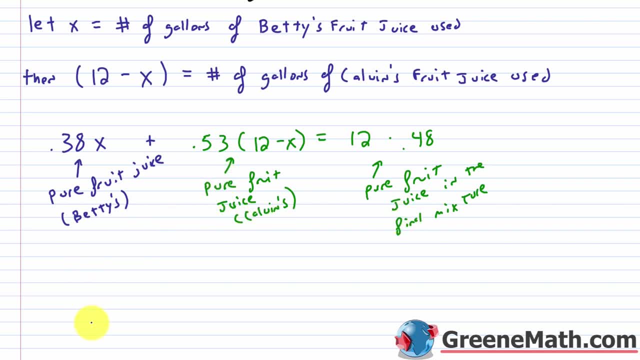 So this has to be true. So once we have our equation set up and we understand the logic behind it, we just need to solve it. we will figure out what x is. that will tell us the number of gallons of Betty's fruit juice used. 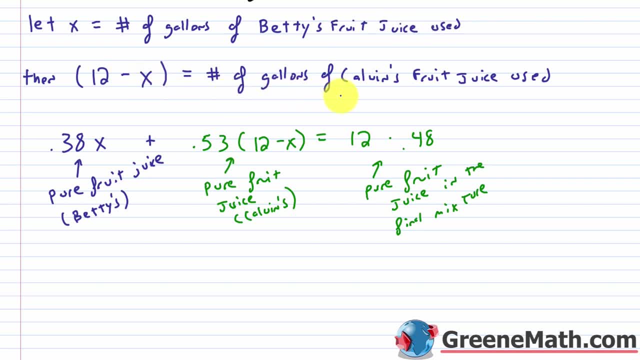 We can then plug in for here and find out the number of gallons of Calvin's fruit juice used, And we've solved our problem All right. So to solve this, we'll have 0.38 times x plus if I use my distributive property. 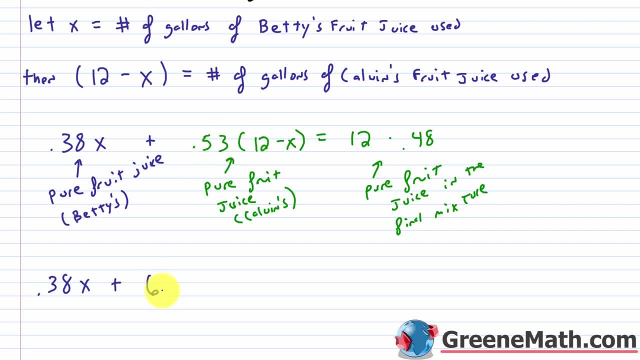 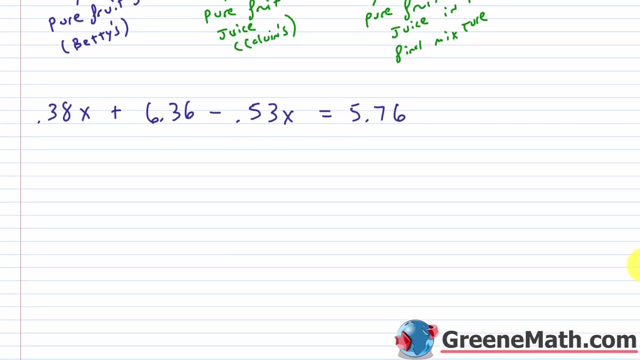 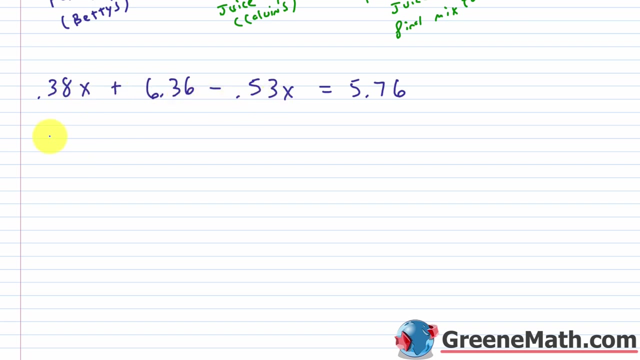 0.53 times 12 is going to be 6.36, then minus 0.53 times x is 0.53x, and this equals 12 times 0.48 is 5.76.. All right, So if we combine like terms here, 0.38x minus 0.53x is negative 0.15x. 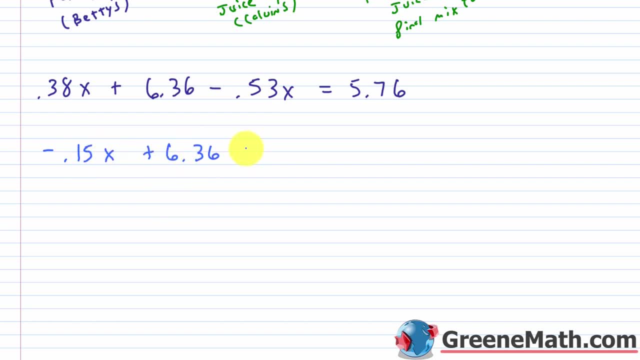 and then we have plus 6.36, and this equals 5.76.. Of course, I will subtract 6.36 away from each side of the equation. So that's gone And I'll have negative. 0.15x is equal to 5.76 minus 6.36. 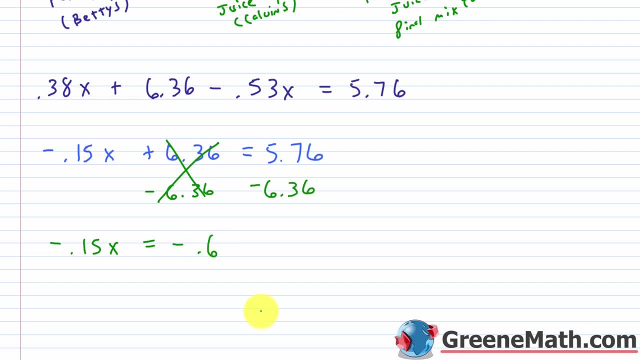 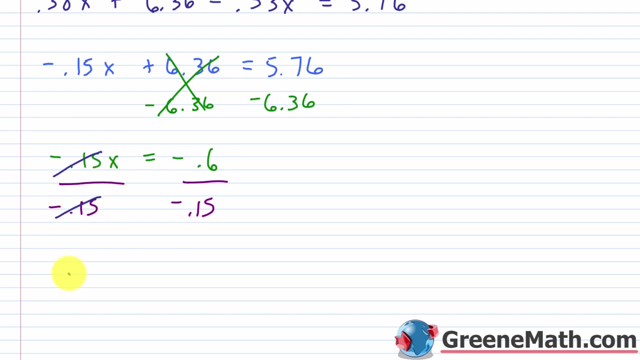 is equal to negative 0.6.. So now, as a final step, we divide both sides of the equation by negative 0.15.. And what's going to happen is this will cancel with this and I'll just have x, and that's equal to negative over negative is positive 0.6 divided by 0.15 is 4.. So x here. 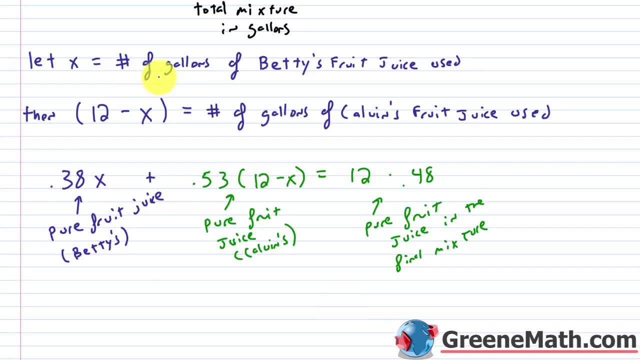 equals 4.. Now, so remember, x was the number of gallons of Betty's fruit juice used. So we're going to use 4 gallons of Betty's fruit juice and then 12 minus 4, or 8 gallons of Calvin's. 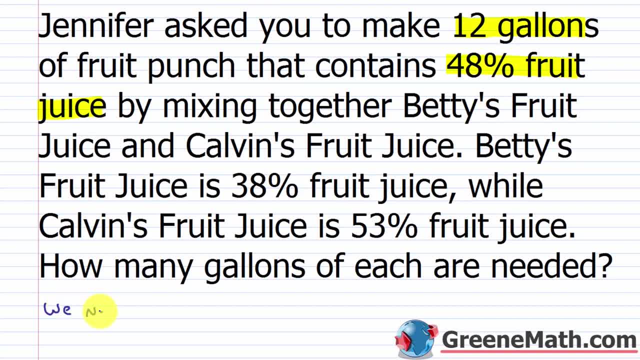 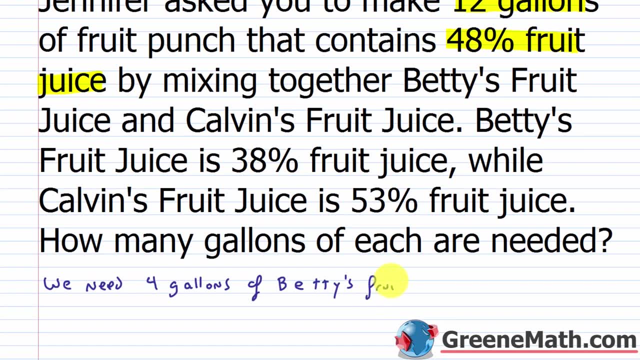 fruit juice. So we can say we need 4 gallons of Betty's fruit juice along with 8 gallons of Calvin's fruit juice. Alright, here we go. implementation again: We have 25 gallons of Betty's fruit juice along with 1.287 times 10,000 of Calvin's fruit juice class. we're�� to do a double. cemos From this is equal to 20 more gallons of Betty's fruit juice, That same time x2.. I wanted to work this the same way. I did old a little bit. here You're still saying the 5.6?. 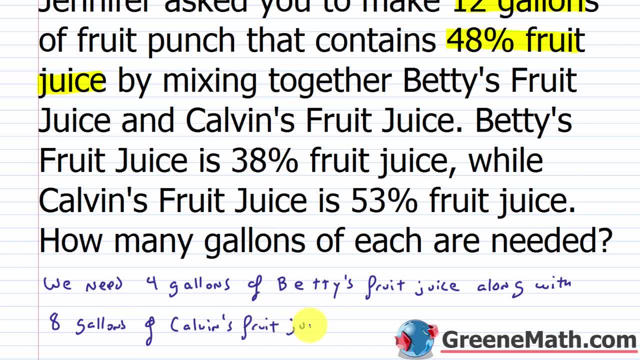 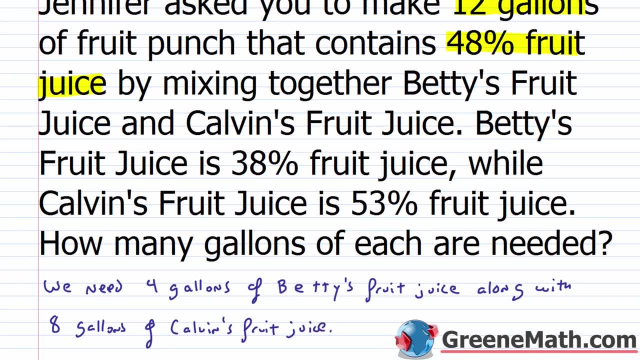 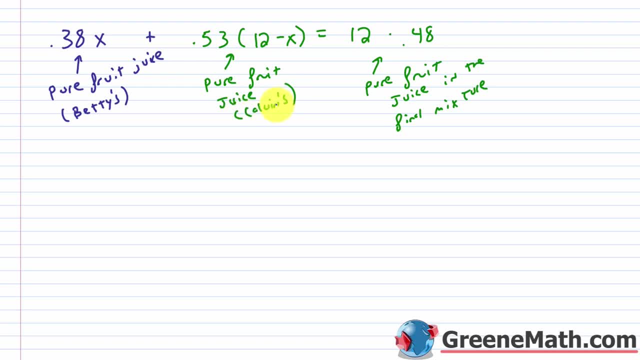 fruit juice and to check this we would think about our equation that we set up. let's scroll down a little bit and again, the amount of pure fruit juice from betty's fruit juice plus the amount of pure fruit juice from calvin's fruit juice has got to be equal to the amount of pure 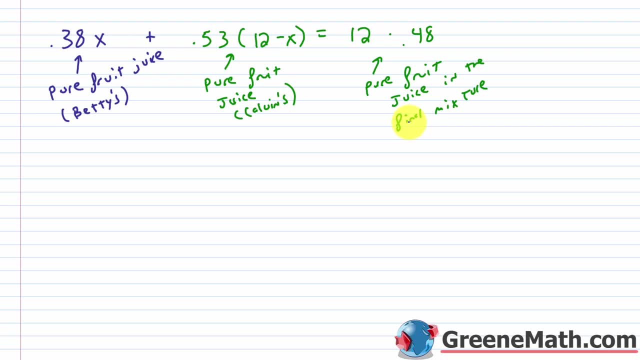 fruit juice in the final mixture. so if i just plug in a four, everywhere i see an x- i can just make sure the left and the right side are equal and i'm going to be good to go. so 0.38 times 4 is 1.52. 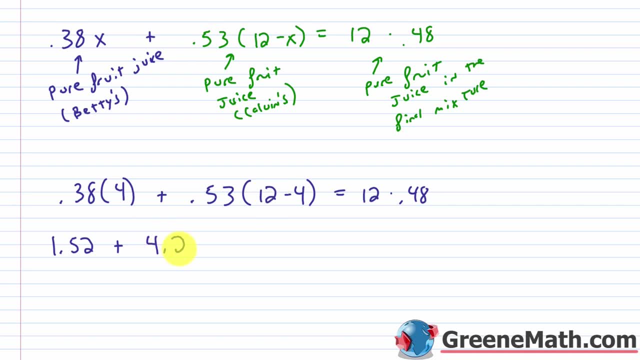 0.53 times 8 is 4.24 and 12 times 0.48 is 5.76. now if i sum these two right here, i do get 5.76. so you get the left side equal to the right side, And it's more important here to understand why they're equal. Again, this right. 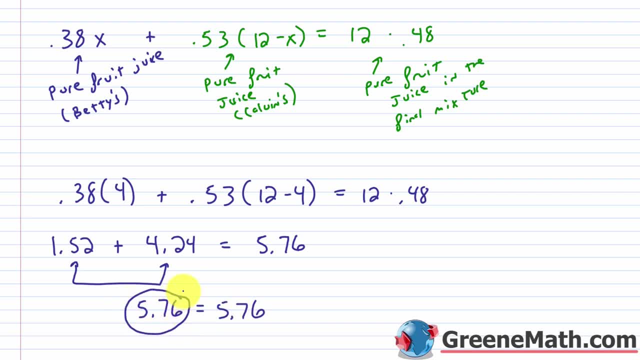 here tells me the total amount of pure fruit juice in gallons that I'm going to have from these two inputs. I've got 1.52 gallons coming from Betty's fruit juice And then I have 4.24 gallons of pure fruit juice coming from Calvin's fruit juice. So again, the sum of that is 5.76 gallons of pure. 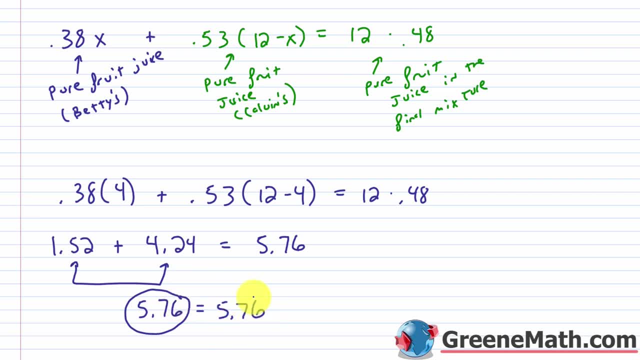 fruit juice And that's what I want. Because of my final mixture here I've got 12 gallons. total, That's 48% pure fruit juice. So it's 5.76 gallons of pure fruit juice in the final mixture. So 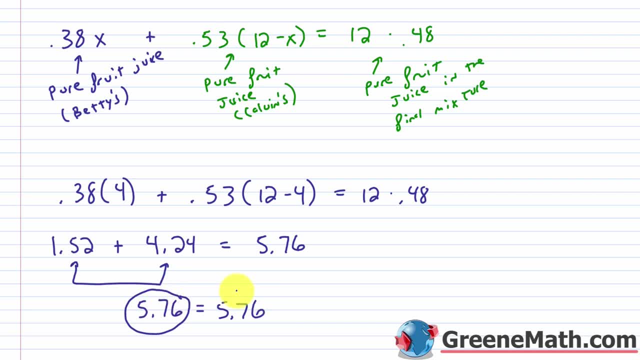 because these two sides are equal. here we know we found the correct answer. Again, we're going to use 4 gallons of Betty's fruit juice along with 8 gallons of Calvin's fruit juice. All right, let's take a look at the next one. So for a bill totaling 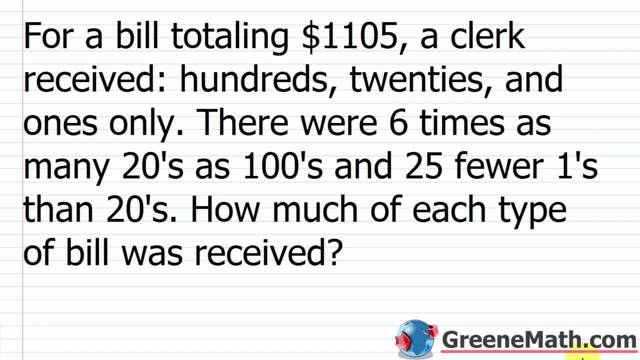 $1,105,. a clerk received hundreds, twenties and ones only. There were six times as many twenties as hundreds and 25 fewer ones than twenties. How much of each type of bill was received? So again for this type of problem? once you read it and you understand what you're being, 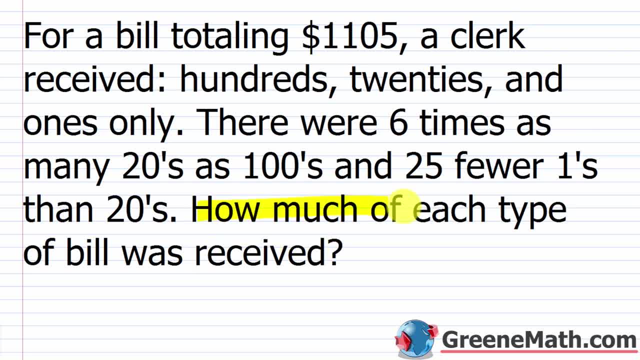 asked, which let's just go ahead and highlight that- how much of each type of bill was received. you're going to be asked to think about what to do in terms of setting up your variable. Now, if you have three things, you need to figure out how many hundreds, how many twenties and how many 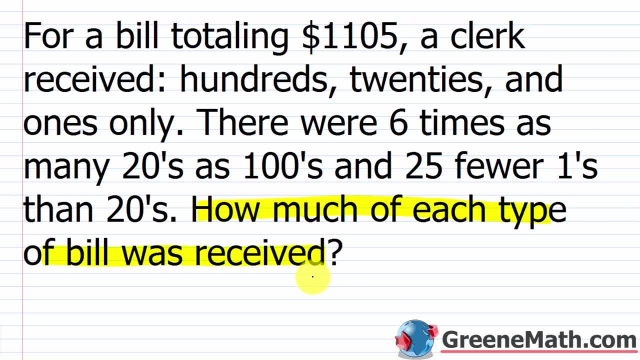 ones. you really need to think about what's going to be easiest for you to use. And again, I keep talking about this in these videos: If you have something that's used in each comparison, then you want to use that, because it's easier to model things. So if we say that there were six times as 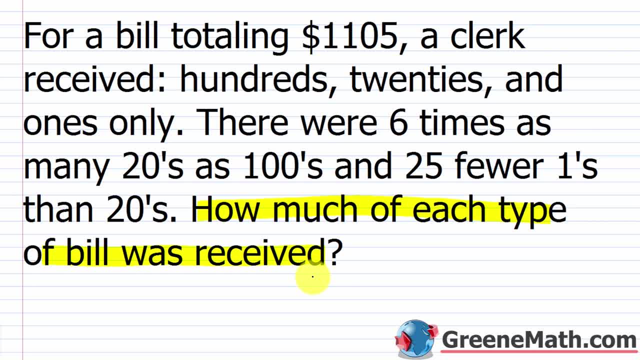 many twenties as hundreds and 25 fewer ones than twenties, then you're going to have to think about how many hundreds, how many ones and 25 fewer ones than twenties. well then, the amount of twenties that were received, or the amount of $20 bills that were received that's used in each. 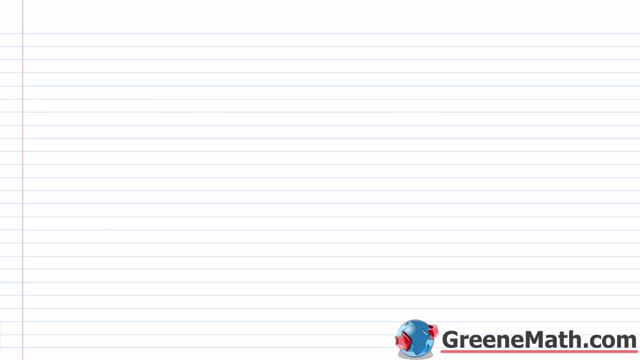 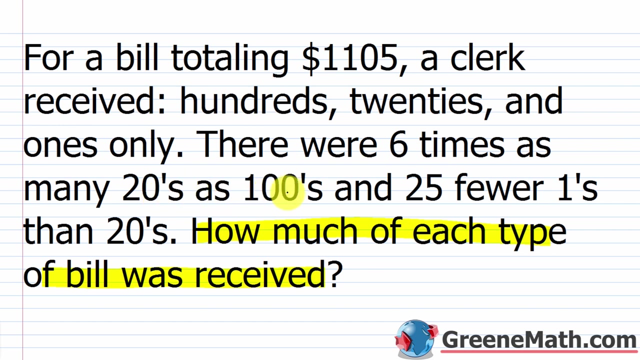 comparison. So it's easiest to just let the variable, like X, be equal to that. So let's let X be equal to the number of twenties received. So then, what can we say about the hundreds? So it says that there were six times as many twenties as hundreds. So that tells me that, when I think 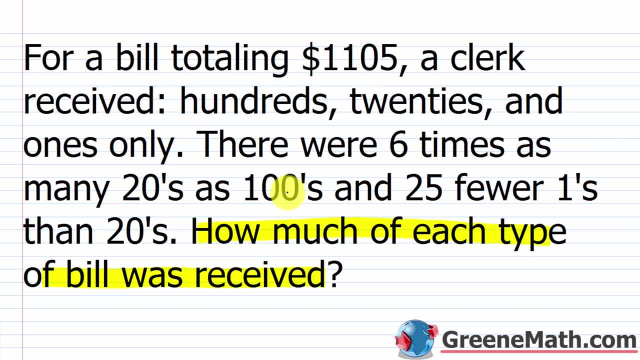 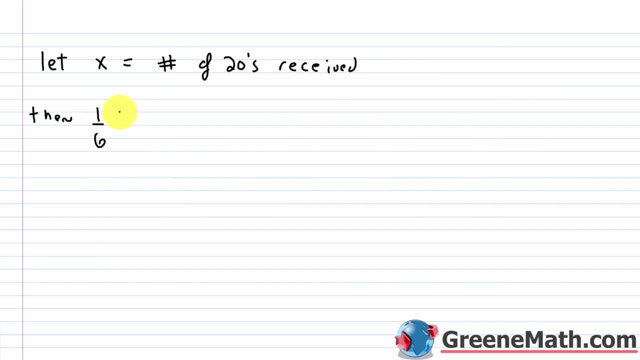 about the number of hundreds, it's one sixth the amount of twenties. So then we can say that one sixth times the number of twenties received, which we represent with X, is equal to the number of hundreds received. Then what can we say about the number of ones? Well, it says that there were. 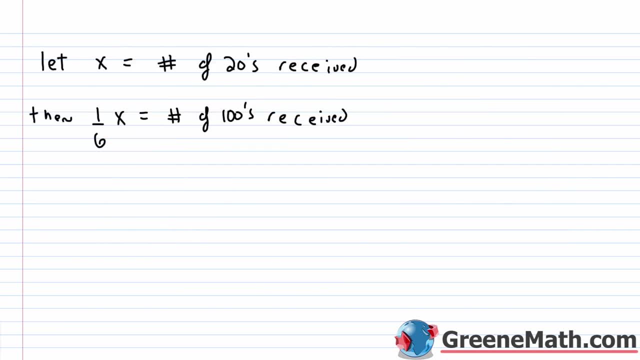 25, fewer ones than twenties. Well, if the number of twenties received is represented with X, then we could say: then, literally, X minus 25 would be equal to the number of ones received. So now that we've represented each type of bill, we want to think about making an equation And what it tells us. 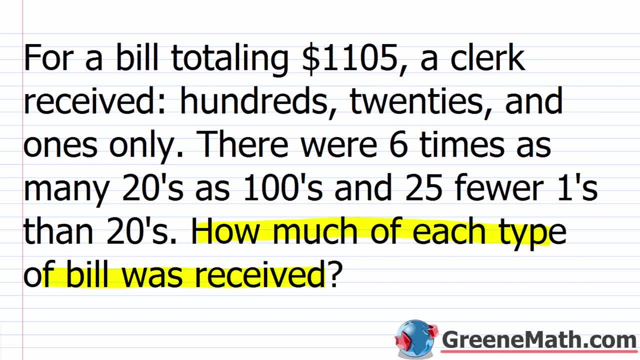 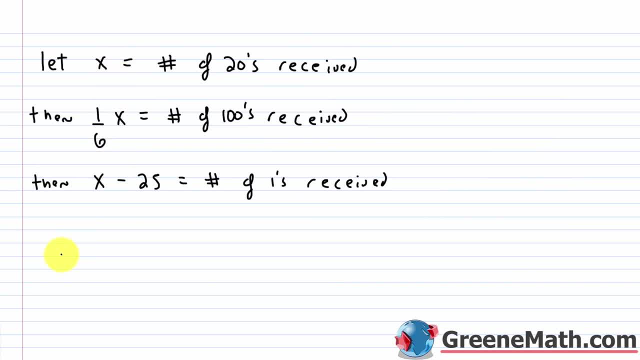 here is that the bill totaled $1,105.. Now, a common mistake with these type of problems is just to take what you modeled here and say, okay, well, X plus one sixth, X plus X minus 25 is equal to $1,105.. That's not going to get you there because, remember, this is a value. This is the value. 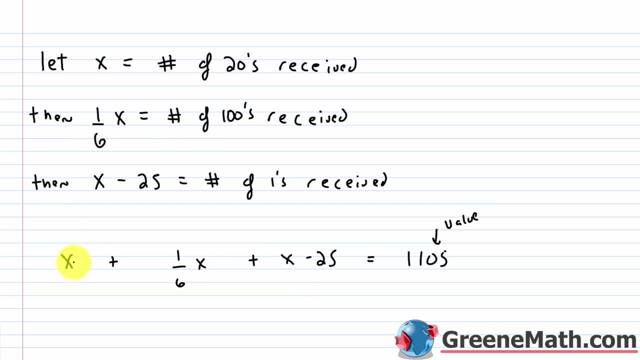 This right here gives you the quantity of bills in each case. X gives you the number or the quantity of $20 bills received. That's just a number. If I hand you four $20 bills, that's not a value. You're just saying, hey, I have four of them. You've got to multiply the four times the value. 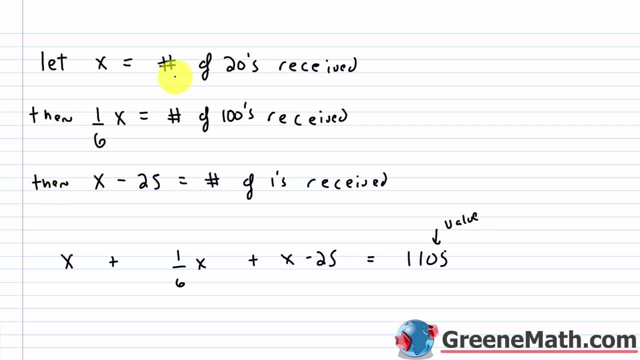 per bill. If it's twenties, then four times 20 would give you 80.. I've got $80.. So you've got to match up the information on the left with the information you're given on the right. So for each type of bill, you got to multiply by the value. So for the twenties, which is 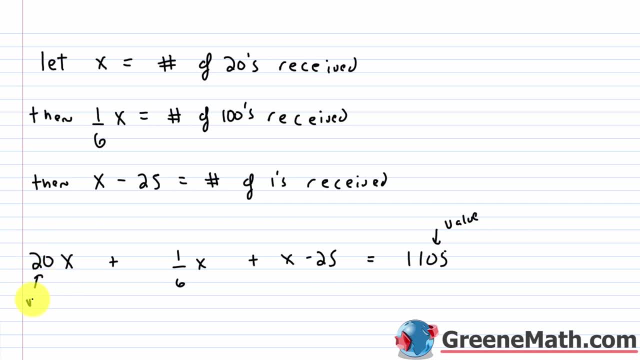 represented with X, I'm going to put 20 next to it. So this is the value and this is the number of bills. Again, I go back to the example. If I hand you four $20 bills, if you plugged in a four there, four times 20 would give you 80. You know. 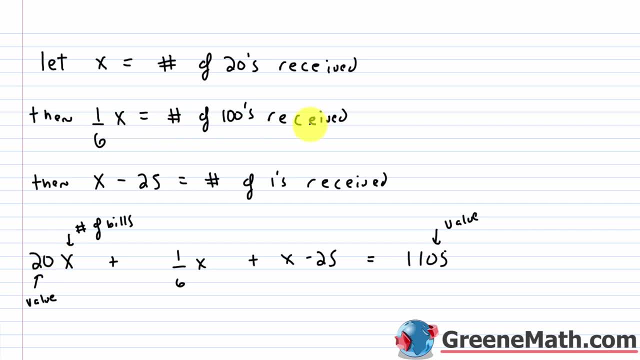 you have $80 there. For the number of hundreds I've got one, sixth X. multiply that by a hundred. And for the number of ones I've got X minus 25, that quantity- make sure you use parentheses- Let's multiply that by one. 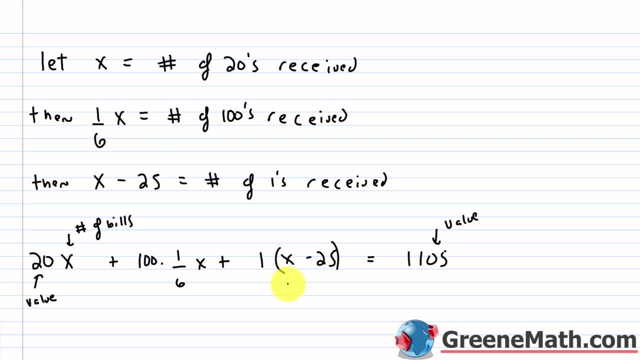 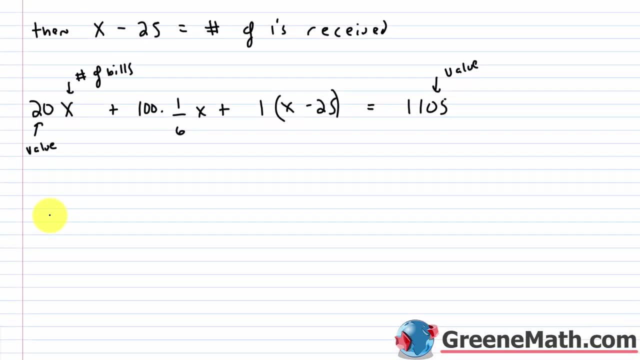 Okay, By one. And you know, one times anything is just itself. but again you want to just use parentheses, So you get in a good habit of things. All right, So now let's solve this equation. We would have 20 X plus 100 times one. sixth. 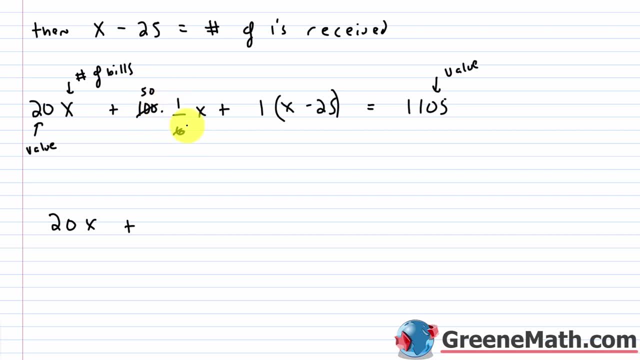 Well, we know they're each divisible by two. This would be 50.. This would be three. So let's put 50 over three times X, then plus- I can just drop the parentheses here- This is just X minus 25.. 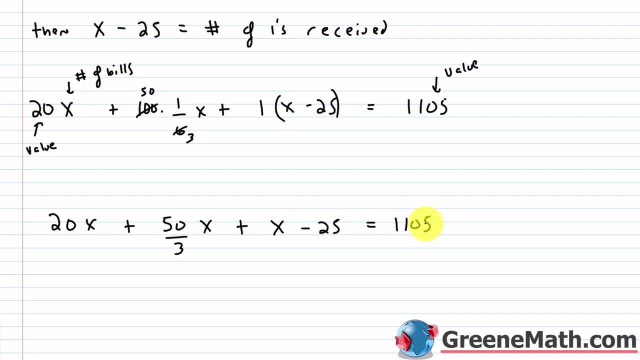 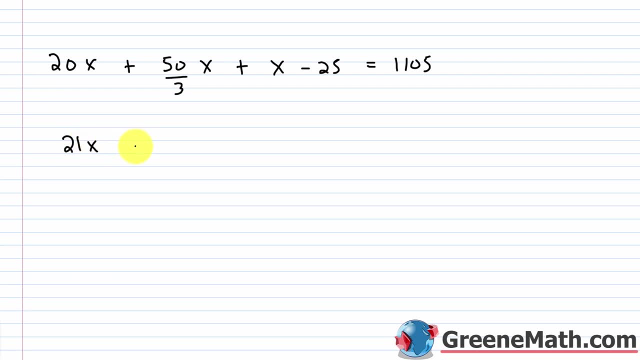 This equals 1,105.. All right, Let's scroll down a little further. So 20 X plus X is 21 X, And then we have plus 53 X, and then minus 25 equals 1,105.. Let's add 25 to each side of the equation. That will cancel and we'll have 21 X plus 53. of 1,100.. igual to 2,500 plus 1,100, and that's 51 X plus 2,500.. That's 51 X plus 2,000.. That's 525.. That's 525.. 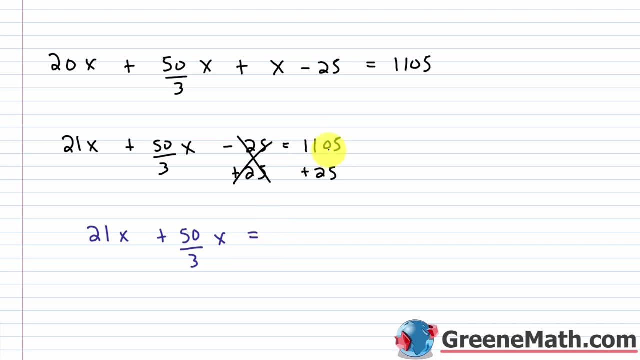 That's: 525 equals 2,100.. x is equal to 1105, plus 25 would be 1130.. I've got a fraction here. I can multiply both sides of the equation by three. Or what I can do is I can multiply this by three over three. 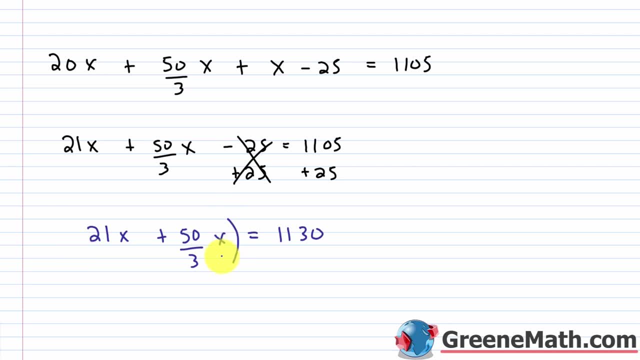 and I can just work with the fractions. It doesn't matter, Typically we just clear the fractions. So let's just do that. Let's multiply both sides of the equation by three. three times 21 would be 63. So this would be 63 x plus three times 50 over three will be 50.. So this would be. 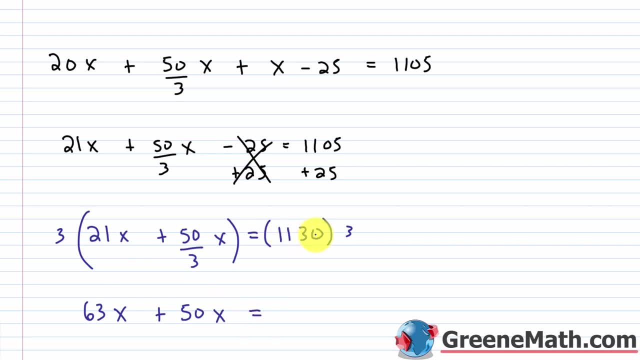 50 x, This equals 1130 times three. Well, if I think about three times 1000, that's 3000.. Three times 100 is 300.. Three times 30 is 90.. So that would be 3390.. All right, so let's continue. 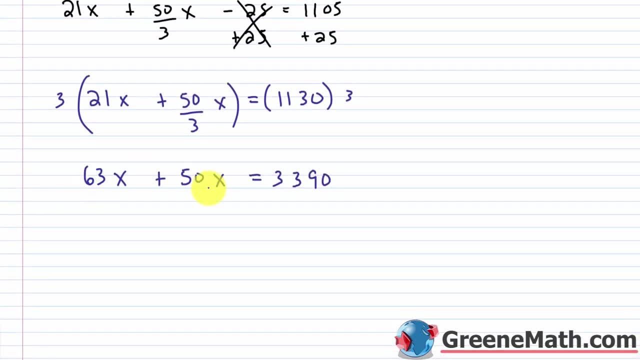 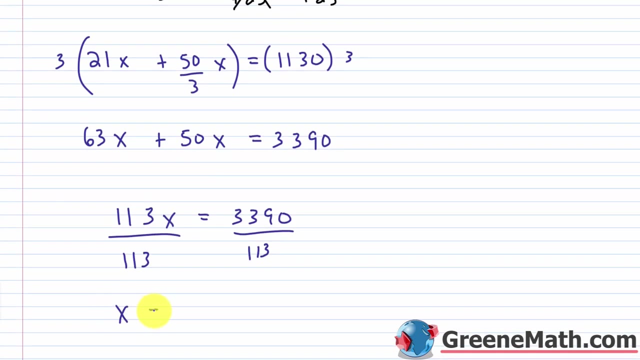 now 63 x plus 50 x three plus zero is 36 plus five is 11.. So this would be 113 x equals 3390.. Divide both sides equation by 113.. And we'll find that x is equal to 30.. Okay, this cancels with this and we got. 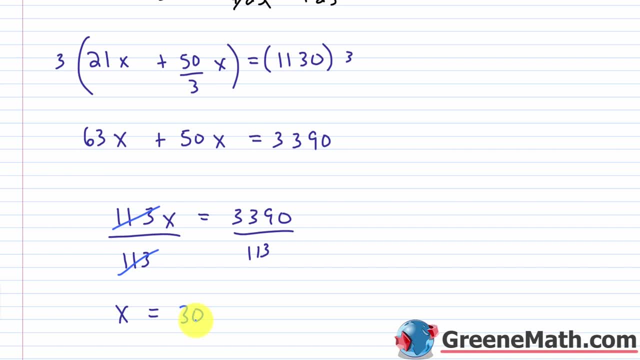 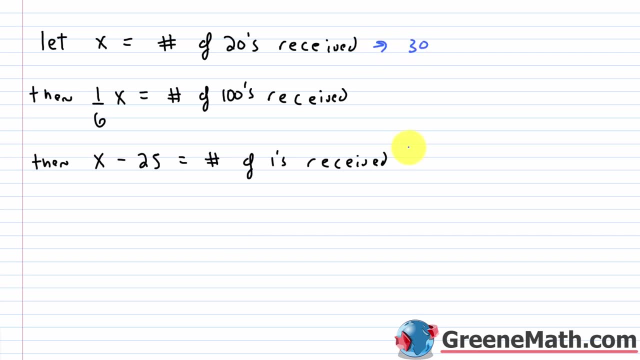 30.. Again, we're working with a word problem. So let's make sense of this Again: if x is the number of $20 bills received and x equals 30, then I know I got 30 of these. And again, if you want to just check things, 30 x 20 would be 600. So the value from the 20s would 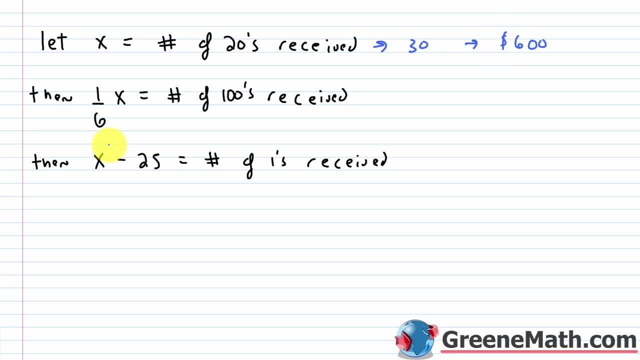 be $600.. Then for the number of hundreds received, it's one six times 30.. 30 divided by six would be five. So they got five of these. the value would be $500.. And then x minus 25 is the number of ones. 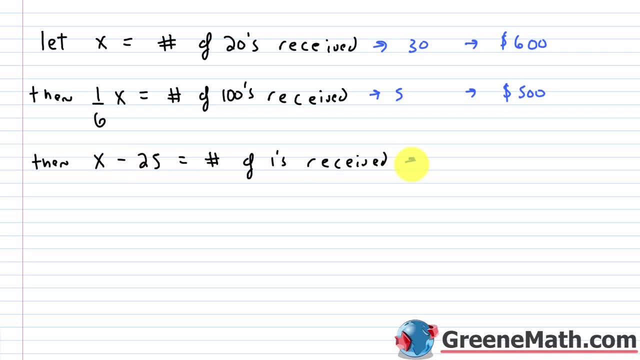 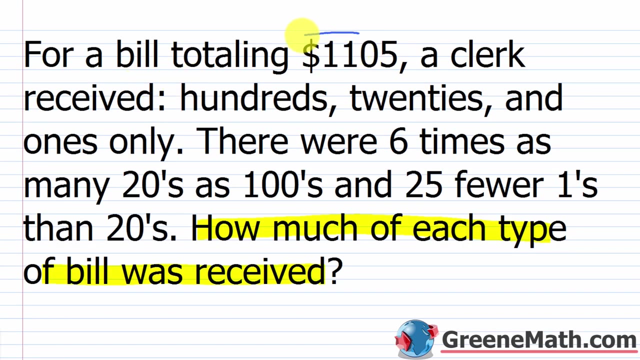 received: 30 minus 25 is five, So this is five, So this would be $5.. And that's consistent with the total. 600 plus 500 is 1100.. 1100 plus five is 1,105.. Again, for a bill totaling $1,105. 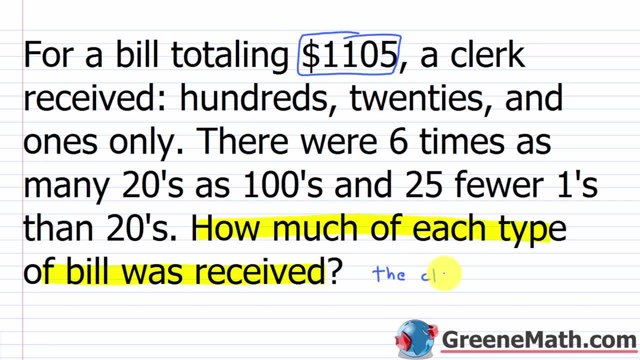 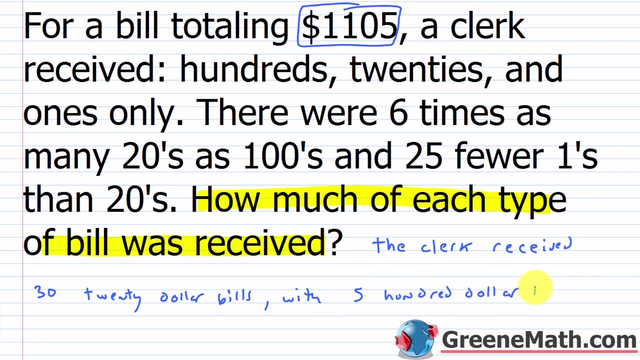 So we can just state that the clerk received 30 $20 bills with five $100 bills and five $1 bills. So again, the clerk received 30 $20 bills with five $100 bills and five $1 bills. And again, easy to check, 30 times 20 is 600.. So that's the value from the 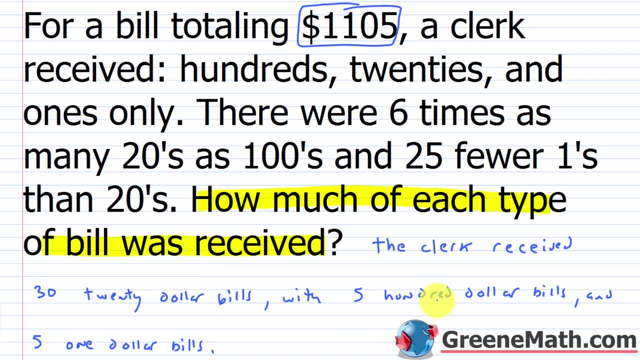 20s received. Five times 100 is 500. So that's the value from the 20s received And again the value from the $100 bills received, And five times one is five the value from the $1 bills. 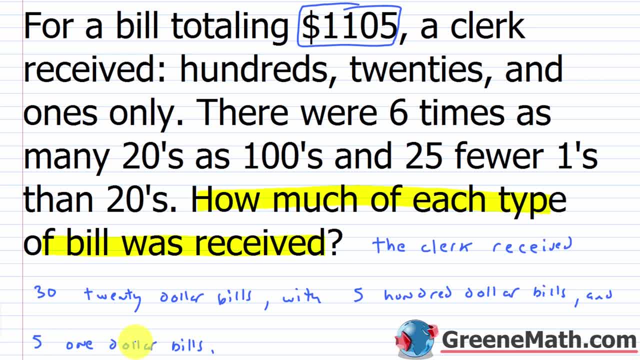 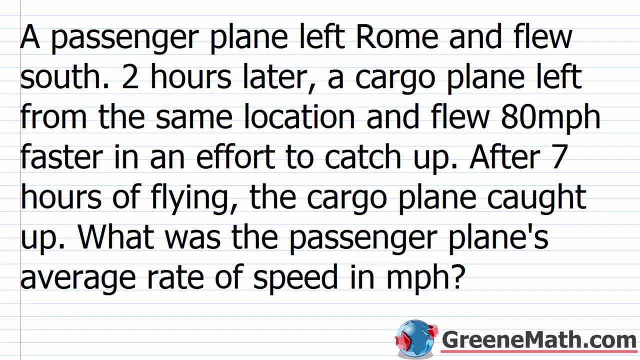 received. So 600 plus 500 is 1100.. 1100 plus five gives you this 1,105.. Again, the total bill that we're told in the problem. All right, so let's take a look at the next one. And now we're going. 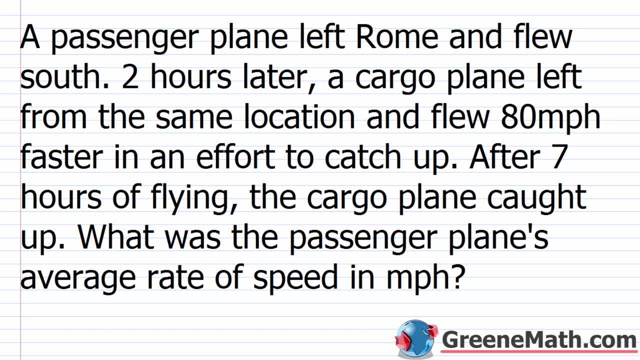 to talk about motion word problems. So we saw these in Algebra 1.. And these use the formula distance equals rate of speed, times time traveled. So if I'm in a car, I'm going to use the formula distance equals rate of speed, times time traveled. So if I'm in a car and I'm going 30 miles an hour, for seven hours. I multiply 30 times seven, that gives me 210. And I know I went 210 miles. So a passenger plane left Rome and flew south. Two hours later, a cargo plane left from the same location and flew 80 miles per hour faster in an effort to catch up After seven hours of flying. 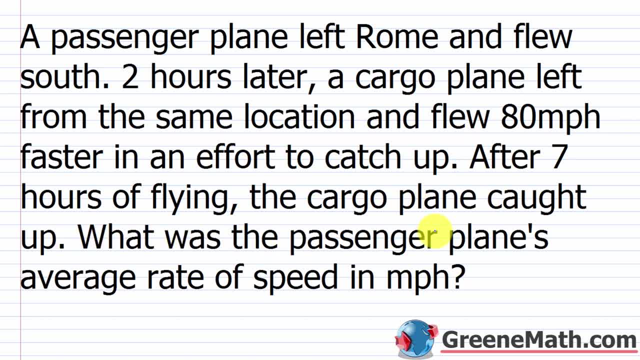 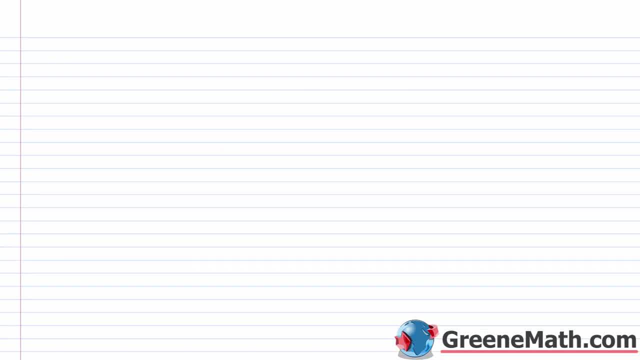 the cargo plane caught up, What was the passenger plane's average rate of speed? What was the passenger plane's average rate of speed in miles per hour? So for this one again, we're going to use our distance formula. So distance is equal to rate of speed, times time. 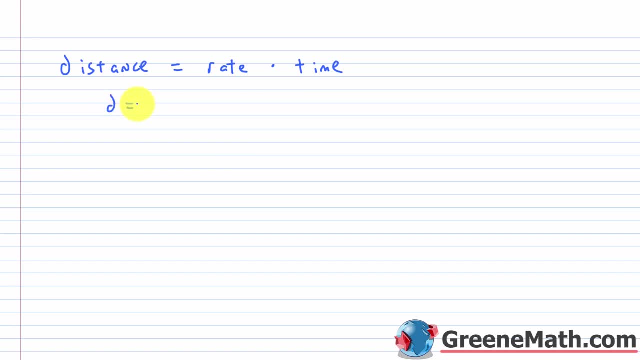 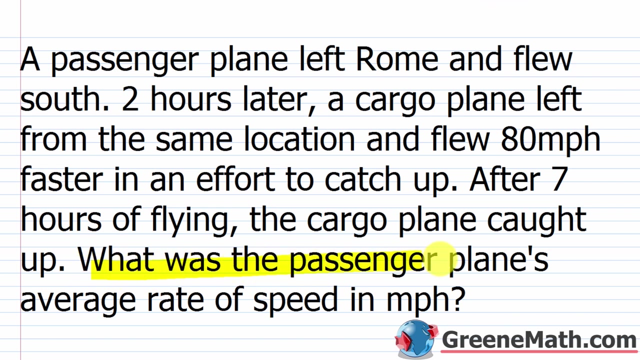 traveled. Okay, this is abbreviated with: D equals R times T. Very common formula, very common type of problem. So the first thing we want to do again, let's go back up. We understand that. the question here is: what was the passenger plane's average rate of speed in? 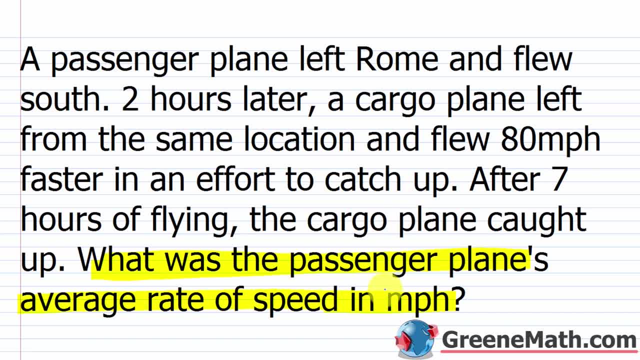 miles per hour. Now, to get this, first we need to figure out what we need to do to model this, And typically you'll say: let's, let x be equal to what you're looking for. Well, we're looking for. 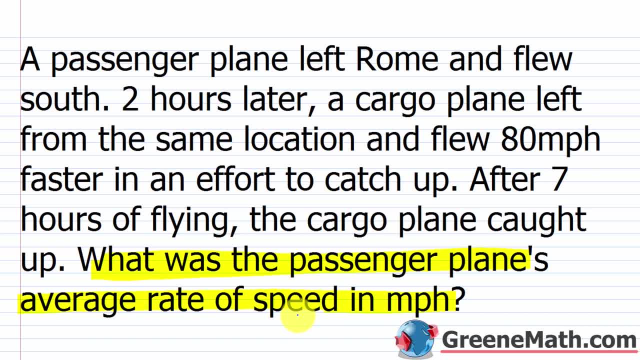 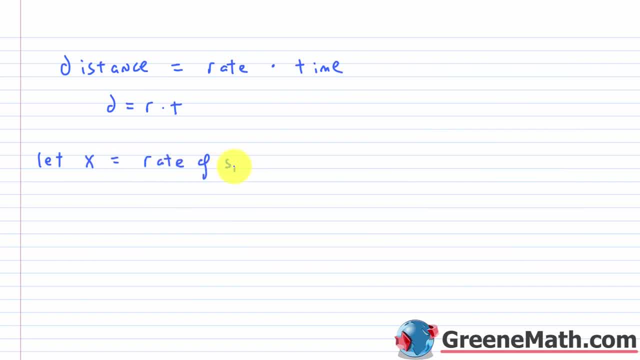 again the passenger plane's average rate of speed in miles per hour. So let's do that. So let's let x be equal to the rate of speed, OK, So once we've established that, let's talk about the cargo plane's rate of speed. So what does it tell us about that? Well, it tells us that the cargo plane left from the same location and flew 80 miles per hour faster. It doesn't tell us anything about the cargo plane's rate of speed, But it does tell us that if we split this chocolateyで. 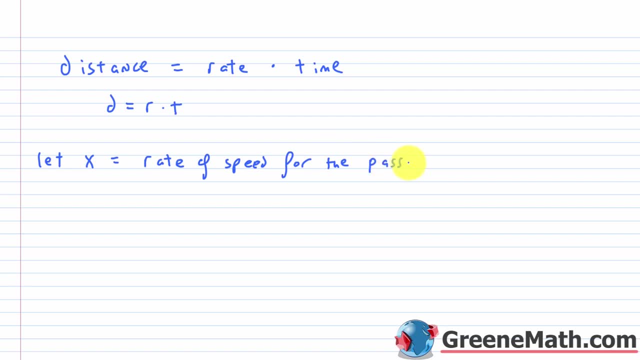 weight of it over horizontal. the cargo planes' rate of speed. their passenger plane's rate of speed is equal to the cargo plane's rate of speed, And that's why we know that Logitech and NodeST form has a breathing target. Okay, so once we've established that, let's talk about the cargo plane's rate of speed. 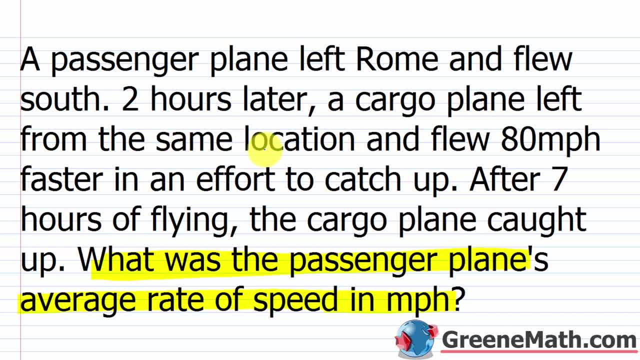 So what does it tell us about that? Well, it tells us that the cargo plane left from the same location and flew 80 miles per hour faster. It doesn't tell us its exact rate of speed, but however fast the passenger plane is going. 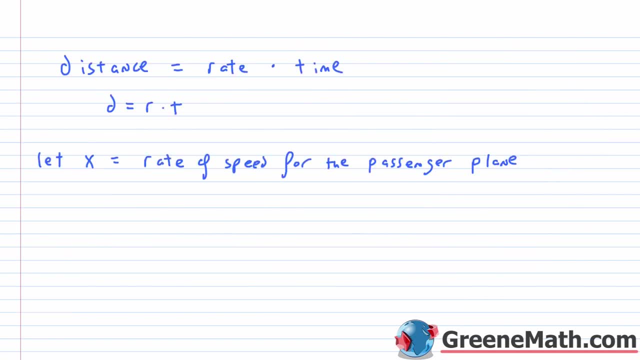 the cargo plane is going 80 miles per hour faster. So then I can say: then x, which is the rate of speed of the passenger plane, plus 80, would be equal to the rate of speed for the cargo plane. So you might be thinking: okay, we've got this kind of setup. how in the world are we? 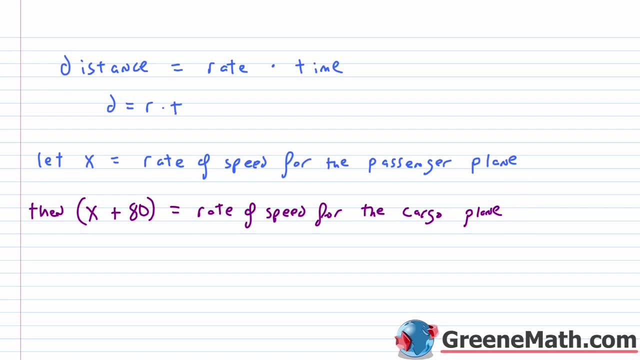 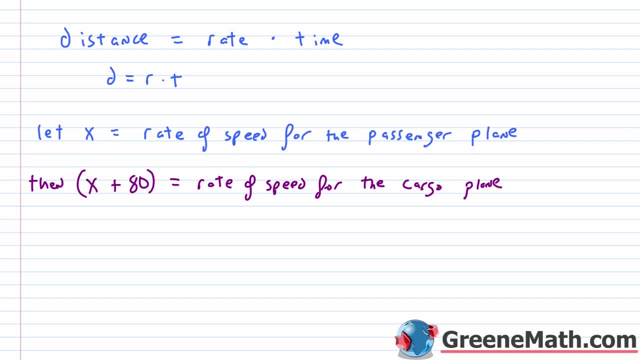 going to get an equation going. Well, what do we do? What do we know here? Let's make a little table. I often don't make tables because in a lot of cases you don't need them, but with a motion word problem, they really help you organize things. 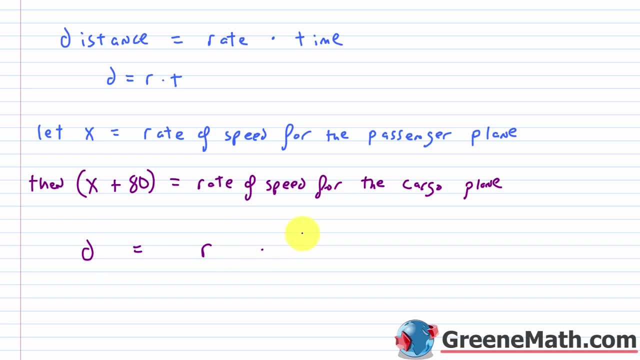 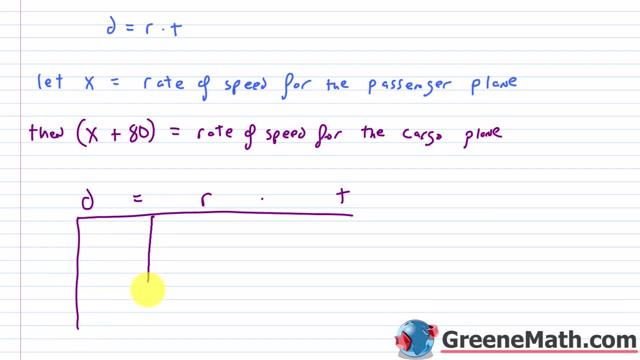 So let's do: distance equals rate, times, time like this. Make a nice little table. We have two scenarios: We have our passenger plane and we have our cargo plane. Now, the rate of speed we know already for the passenger plane, the r we've modeled. 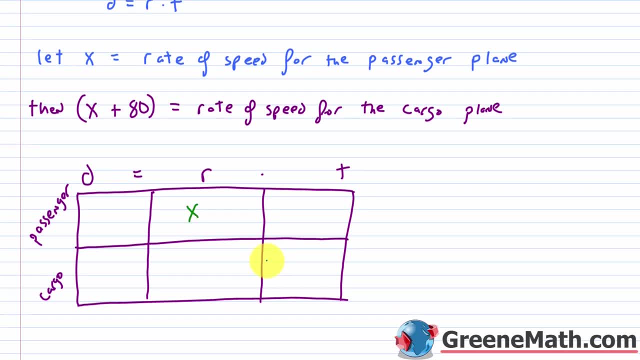 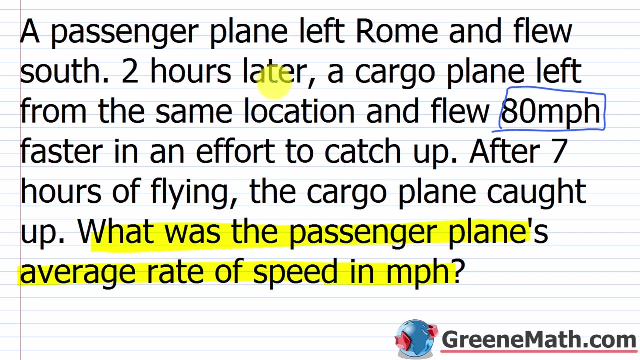 it with x. That's easy enough For the cargo plane. we know it's x plus 80.. Now does it say anything in the problem about the time? No, Well, yeah, it kind of does. A passenger plane left Rome and flew south two hours later. 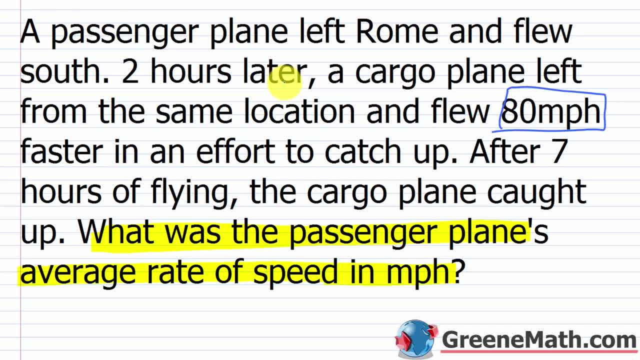 So that means that the passenger plane is traveling for two hours more than the cargo plane does. So two hours later, a cargo plane left from the same location and flew 80 miles per hour faster in an effort to catch up After seven hours of flying. so let me just stop there. the cargo plane flies for seven. 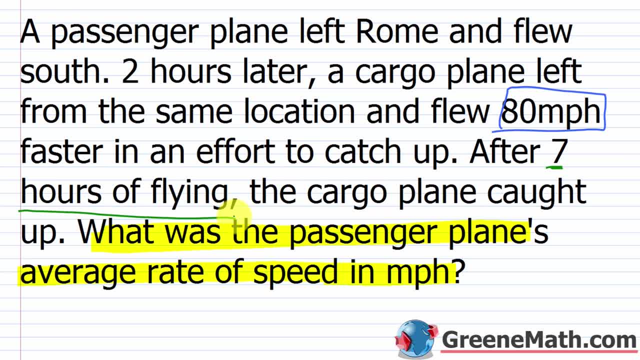 hours. The passenger plane: again, it tells us, because of this two hours later thing, here was flying for a total of nine hours. So nine hours for the passenger plane, two hours less for the cargo plane, seven hours. Let's go back down. 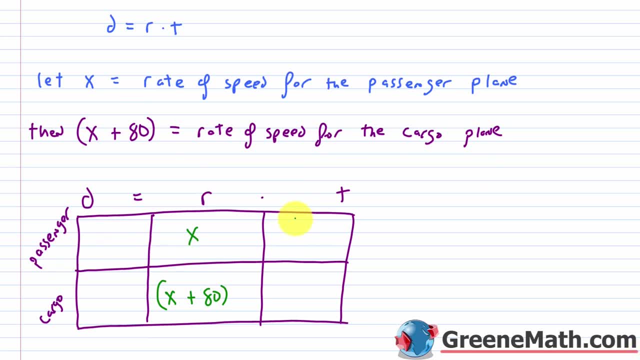 Let's fill in the information here: For the passenger plane, it's nine hours, For the cargo plane it's seven. Now I want you to realize something: They didn't tell us a distance, But if I have a plane, I can tell you a distance. 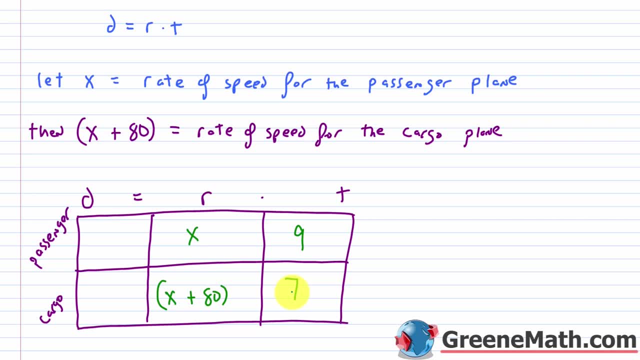 But if I have a rate of speed and I have a time, I have a distance, because I just multiply the two together. If my rate of speed is 30 miles per hour and my time is seven hours, 30 times 7 is 210,. 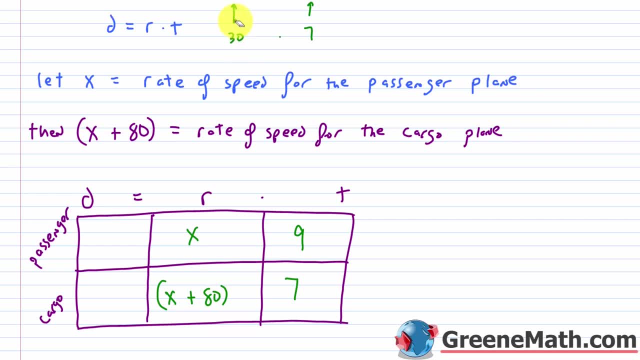 I know my distance Right. It's 210 miles. in that case It's the same thing here. I have a rate times a time, So 9x is the distance. I have a rate times a time, So 7 times the quantity x plus 80.. 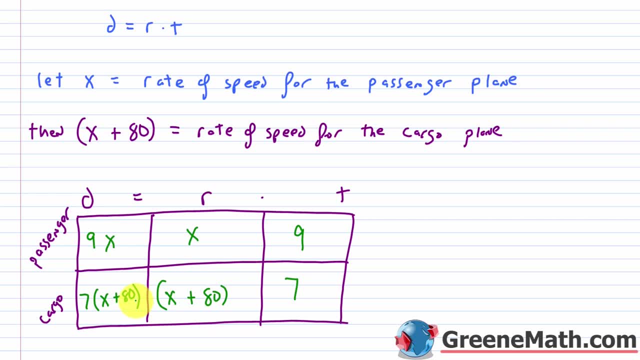 Okay, So 7 times the distance, And you might say, okay, well, that's great. How do we get an equation? Well, there's one thing that you might have missed out on here. Let me go back up And let's read through the problem one more time. 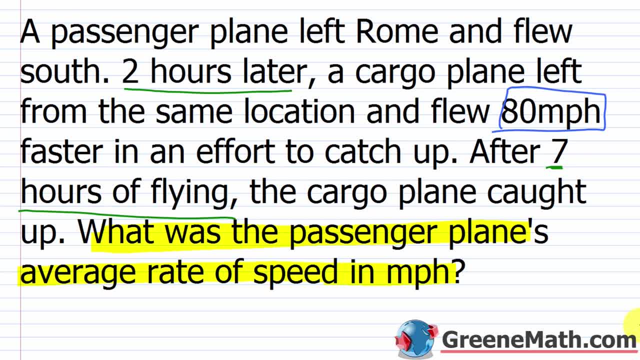 What could you see? that's equal. here Again, a passenger plane left Rome and flew south. Two hours later, a cargo plane left from the same location. So they leave from the same location And flew 80 miles per hour faster than a passenger. 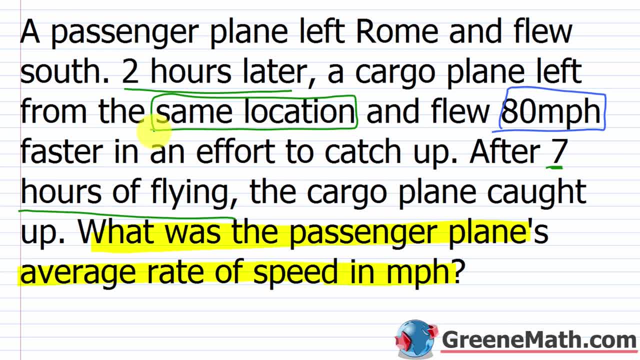 And flew south And flew south to catch up. after seven hours of flying the cargo plane caught up. so that means they end at the same location, they start at the same location, they stop at the same location, where the problem kind of stops at the same location, you might as well say that, but for the sake of the problem they went the. 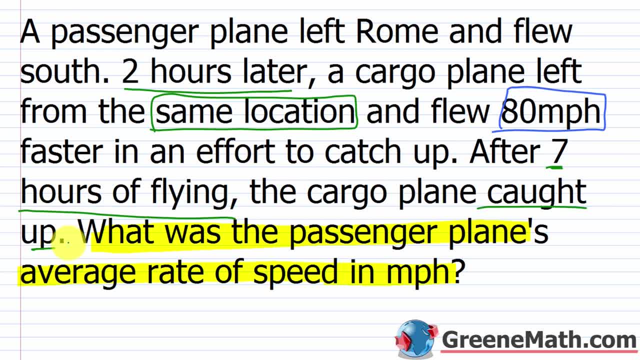 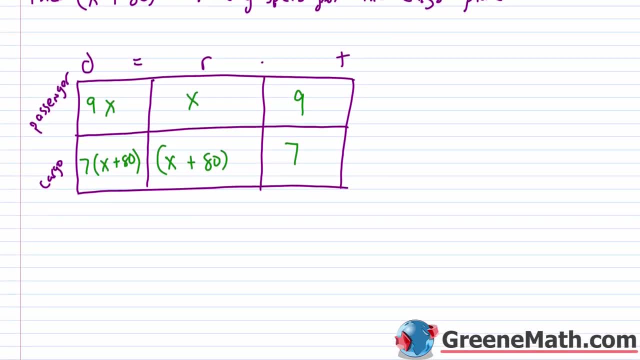 same distance. so that means the distance that the passenger plane went is the same or is equal to the distance that the cargo plane went. now, coming back down here, i know what the distance is for each one. so voila, i've got my equation, because all i have to do is set this distance, which is 9x. 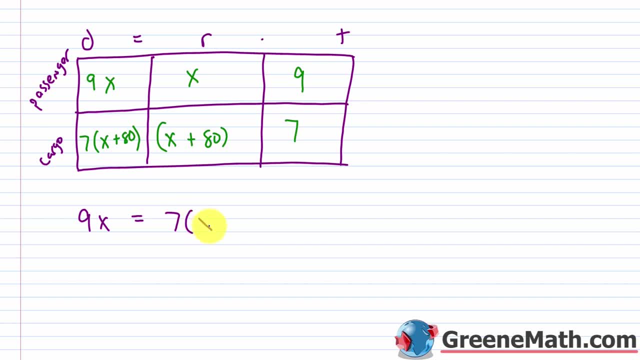 equal to this distance, which is 7 times the quantity x plus 80, and i can solve my equation for x, so use my distributive property over here on the right. 7 times x is 7x plus 7 times 80, which is 7 times. 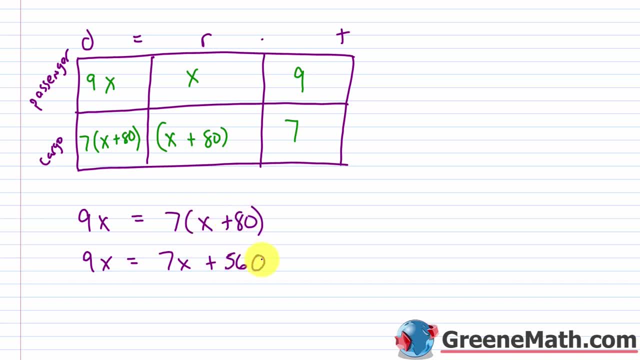 4x 8, that's 56. put a 0 at the end, that's 560.. it would subtract 7x from both sides of the equation. that cancels, you'll have 2x is equal to 560. divide both sides of the equation by 2 and what's going? 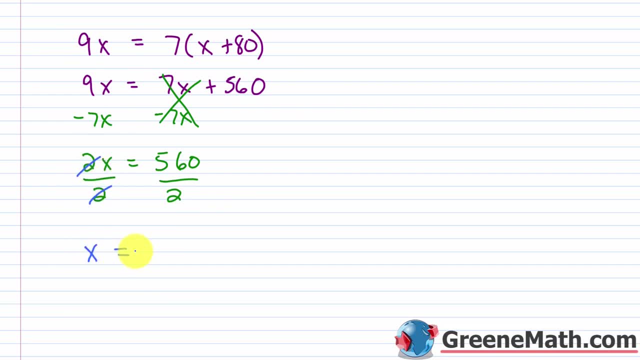 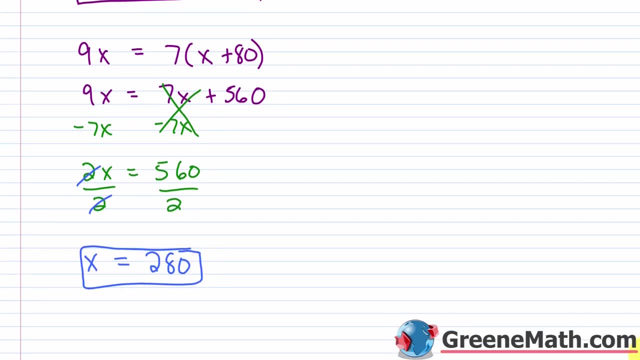 to happen is this will cancel. with this i'll have: x is equal to 560, divided by 2 is 280.. so what does that tell me? let me go back up. x was the rate of speed for the passenger plane, so that tells me that the passenger 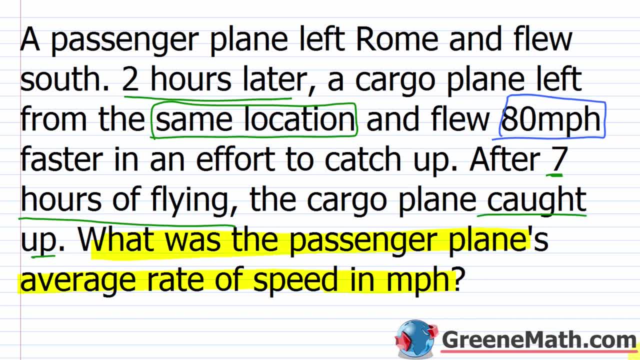 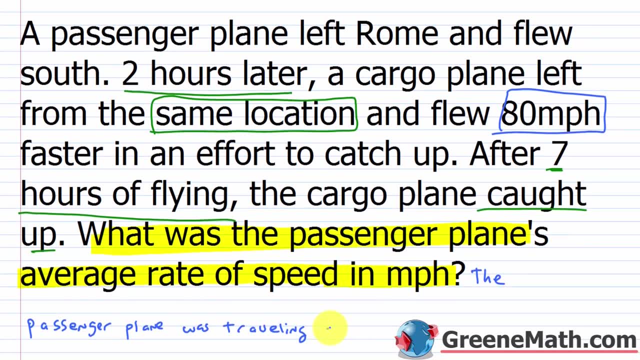 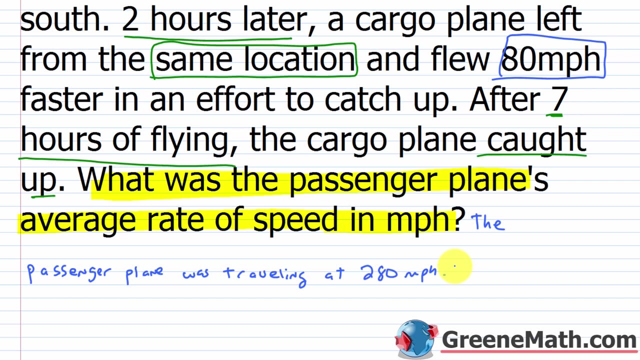 plane was traveling at 280 miles per hour. so the passenger plane was traveling at 280 miles per hour. that's their average rate of speed. how do we check this? well, it's actually pretty easy. if i take 280, which is the rate of speed, and i'm 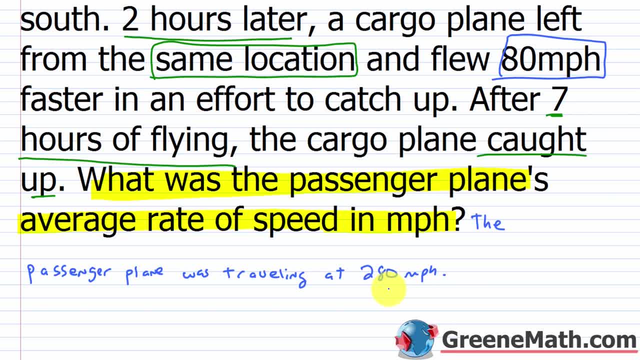 going to multiply it by 9, which is how long the passenger plane travels for, i get 2520. that's the total number of miles that the passenger plane traveled. now, with the other guy, the cargo plane, it goes faster. 280 plus 80 is 360, so that's its average rate of speed in miles per hour it does. 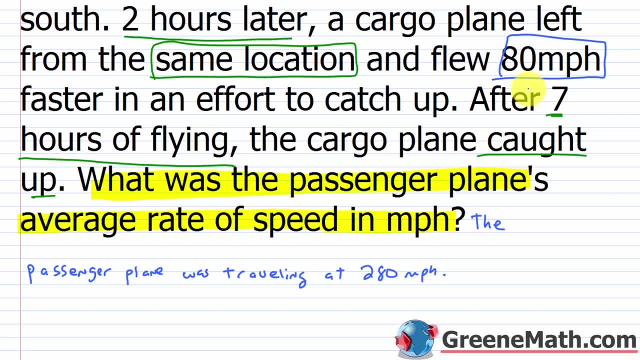 it for seven hours. if you multiply 360 by 7, you also get 2520, so the mileage syncs up there. they traveled the same number of miles, so the distances are equal when we check them, so we know i had the correct answer. the passenger plane was traveling at 280 miles per hour. hello and welcome to algebra. 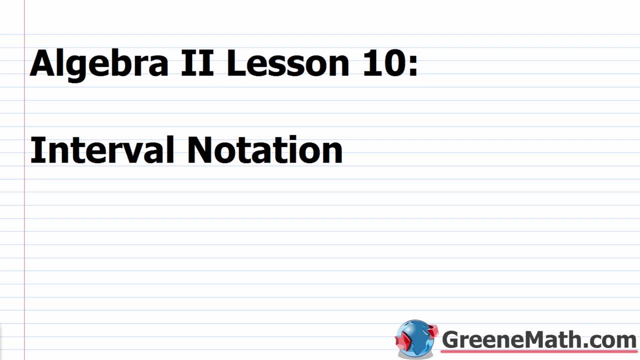 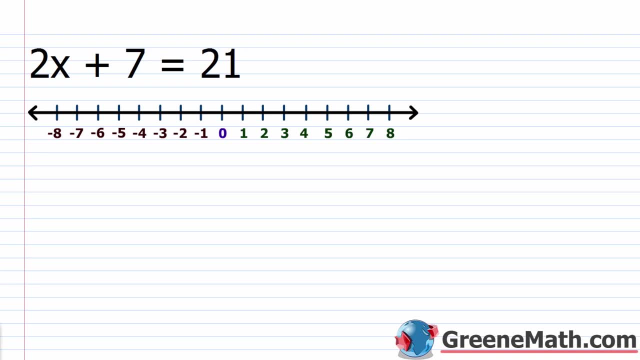 2, lesson 10.. in this video, we're going to learn about interval notation. so, starting on our next lesson, we're going to talk about linear inequalities in one variable, and most of you know from algebra 1 that we have a method to display our solution for this type of problem. 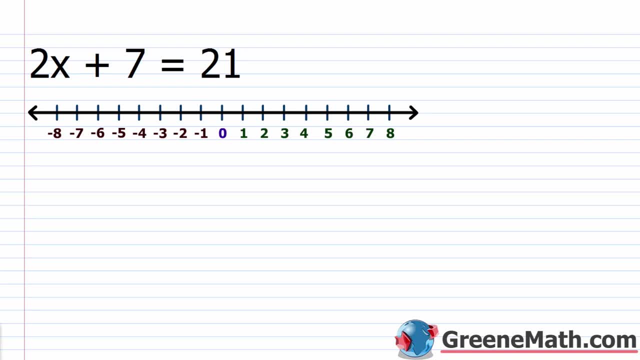 and it's known as interval notation. interval notation allows us to notate a specific range of numbers on a number line. so before we kind of get into interval notation, let's just start out with a typical equation and we'll just show you a few things. so we have: 2x plus 7 equals 21. so we know. 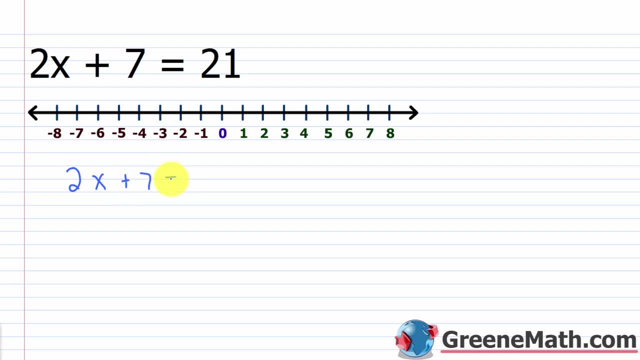 how to solve this at this point. 2x plus 7 equals 21, so we would subtract 7 away from each side of the equation and we would have 2x is equal to 14. divide both sides by 2 and i'll get x is equal to. 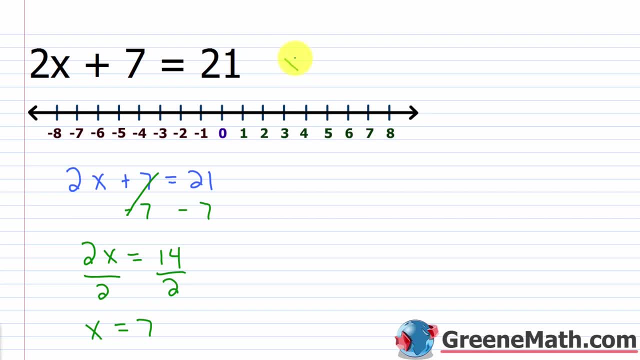 7.. now, normally this is fine. we just put x equals 7.. that's a perfectly acceptable way to notate your solution. you could also use a solution set. so the set contains one element. the element is seven. additionally, we could show the solution graphically. i have a number line here. i could just 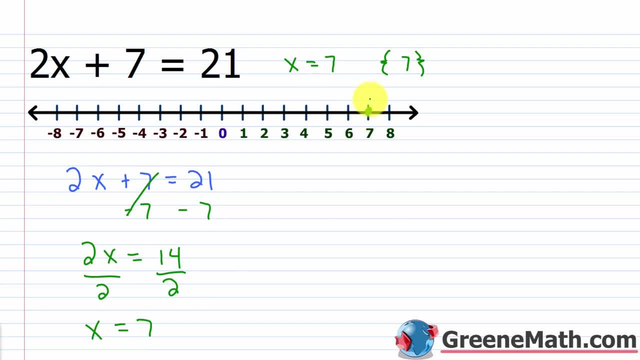 put a filled in circle at seven. so these are all ways i could show the solution for this equation. then there's another one. we're going to talk about this more at the end of this lesson. there's something known as set builder notation. so i could say the set of all elements x, such that x. 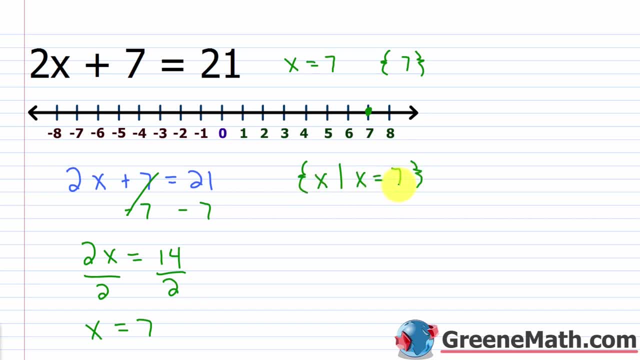 is equal to 7.. and if this doesn't make sense now, that's okay, we're going to cover it at the very end of this lesson. but the point is just to show you that there are many different ways to notate the solution for this equation. 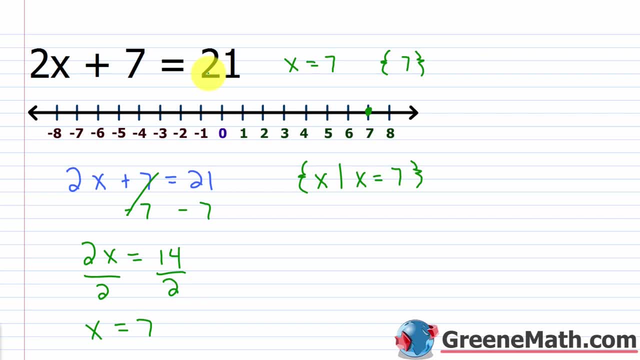 and in every situation. it's basically telling us what that x needs to be replaced with 7 for us to get a true statement. 2 times 7 will be 14. 14 plus 7 is 21.. if i replace x with anything else, 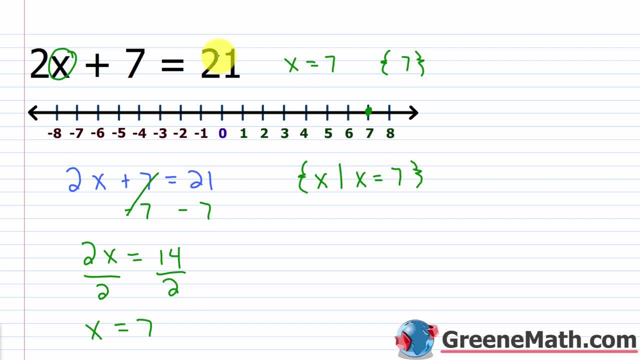 i will not get a true statement right. the equation will be false. all right, so now let's look at an inequality, and it's nothing we have to solve. we're just looking at. x is greater than 7.. so what can i replace x with here? well, it's no longer a single value. 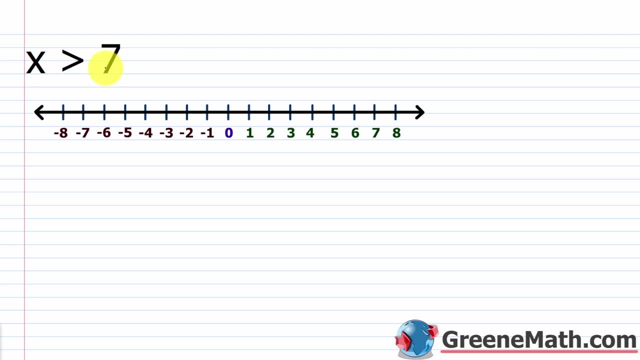 i can replace x with anything that's actually larger than 7.. if i put 7 in itself, it won't work. 7 is not greater than 7. that's false, but anything larger than 7, anything to the right of 7. on the. 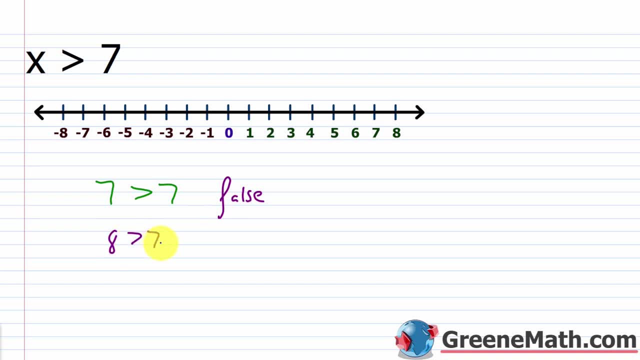 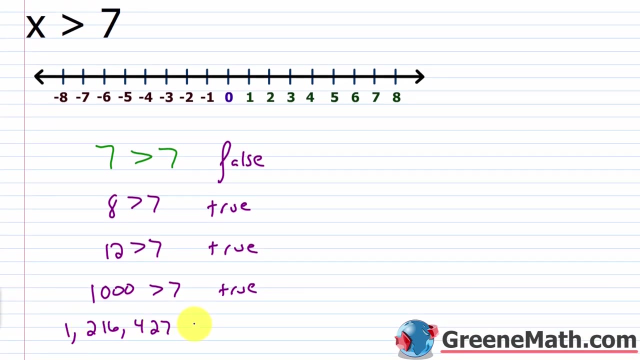 number line would make it true: 8 is greater than 7.. that's true. 12 is greater than 7.. that's true. 1 000 is greater than 7.. that's true. 1 million 216 427 is greater than 7.. that's true. so if i replace x with any value that is larger than 7, 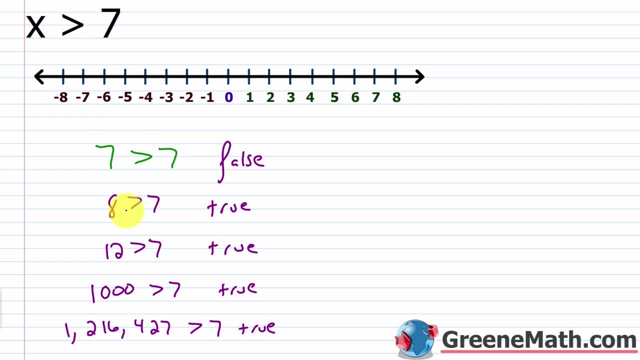 i will get a true statement. so how do we notate this graphically? well, on the number line we would locate 7, and we want to mark 7 as a boundary point or an area that will separate the solution part from the non-solution part. so we do this with two different things. we can either use a parenthesis, 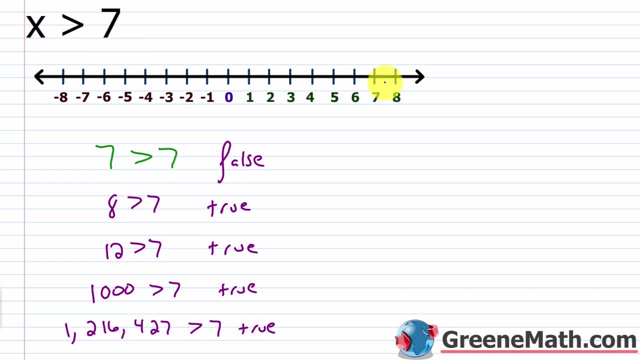 or we can use an open dot. so at 7 i can use an open dot like this, which a lot of students will see that in their class, or i can use a parenthesis that faces towards the solution region. now, since x is greater than the solution, region is to the right of 7.. so i would face my parenthesis to the right. 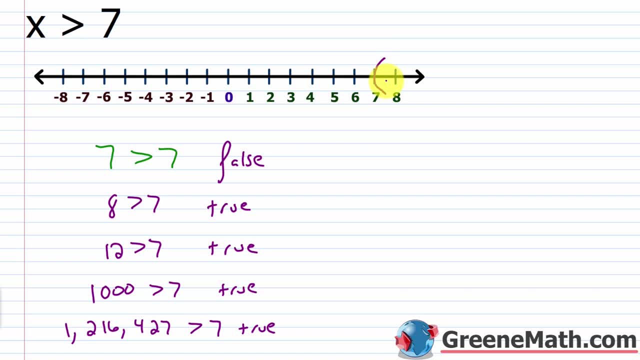 and it would touch 7 like that. now, once we have that, what we want to do is we want to shade the number line again to the right of 7, because that's what satisfies this inequality. so i would shade all of this and i would shade my arrow to say, hey, this continues forever and ever, and ever. 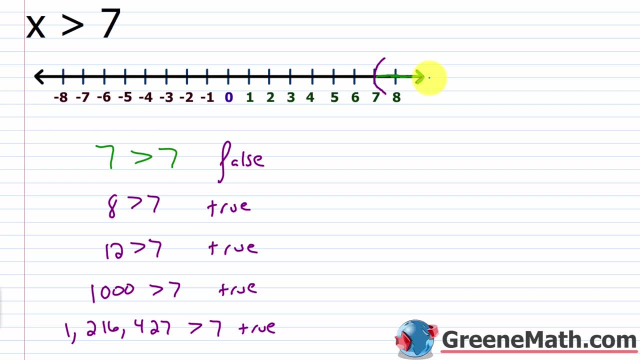 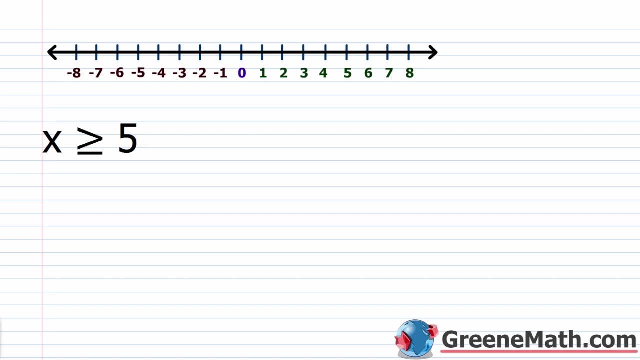 and so any number that is larger than 7 would satisfy this inequality. now, in the situation where you have something known as a non-strict inequality, we use a different variation of this. we would use a bracket or a filled in dot. so, for example, if i replace x with 5, it would be 5 times 5, which is greater than or equal to 5. 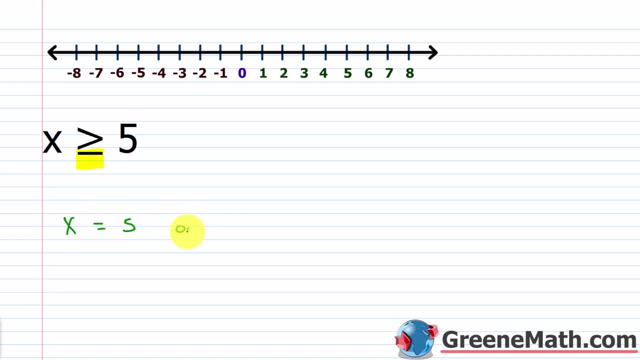 now, because this or equal to remember, x can be equal to 5 or x can be greater than 5 for this to be true. so now, if i replace x with 5, 5 is greater than or equal to 5. that's true because this part. 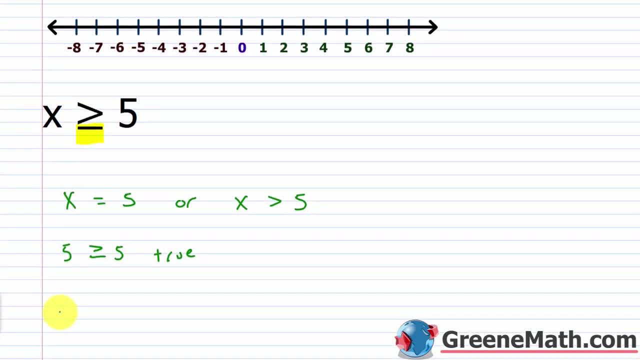 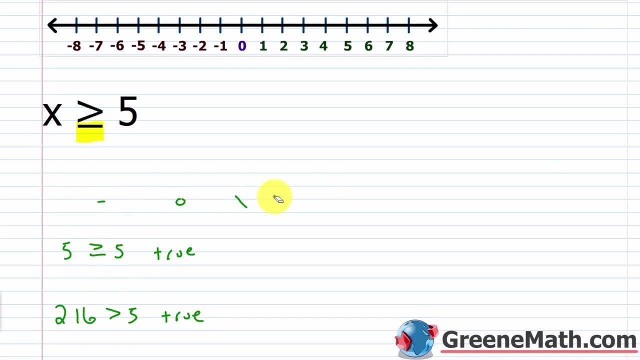 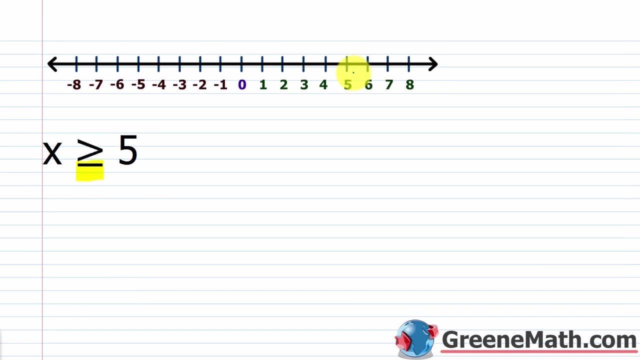 is true. 5 is equal to 5, or any number larger than 5 would also work, if i do- is greater than 5.. That's true. So x can be anything that is again 5 or anything larger than 5.. So, at 5, instead of putting a parenthesis or an open dot, I'm now going to put either a 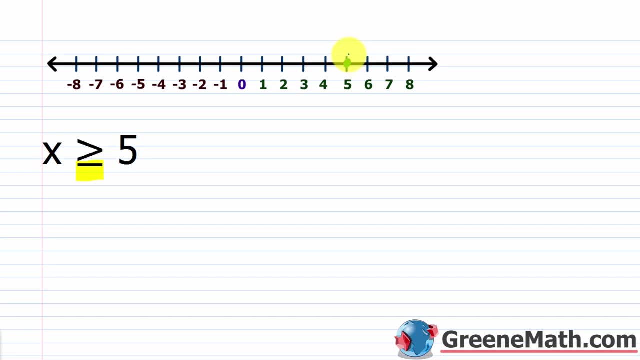 filled in circle or filled in dot, like that, or I'm going to put a bracket there that faces towards the solution region. Again, this is a greater than or equal to, so the solution region is to the right. So I put a bracket here And then, just like I did in the last example, I'm 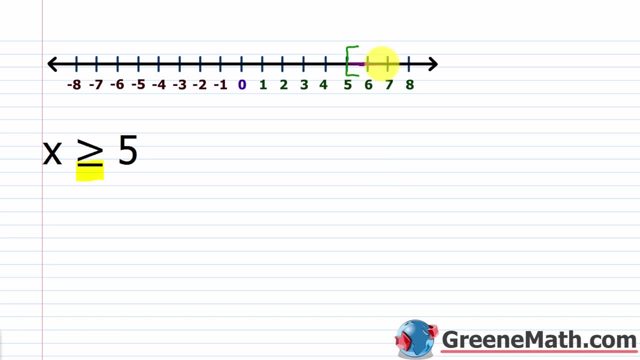 going to shade the solution region. So I'm going to shade everything to the right And I'm going to shade that arrow to say, hey, this continues forever and ever and ever. All right, let's try a few examples here. So if I saw something like x is less than 3,, well, I'd find 3.. And at 3,, 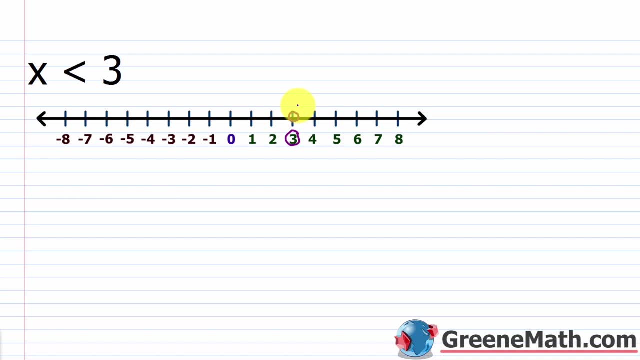 I can either put again. I can put an open dot or an open circle. Got to make sure that there's no color inside of it. Indicate that 3 is not part of the solution, because this is a strict inequality. This is. 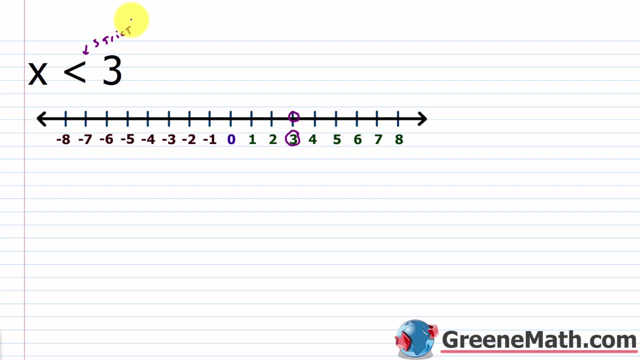 strict x. there cannot be 3.. If I put this here and it's x is less than or equal to 3, well then this would be filled in, because now x can be equal to 3.. But that's not what we have. 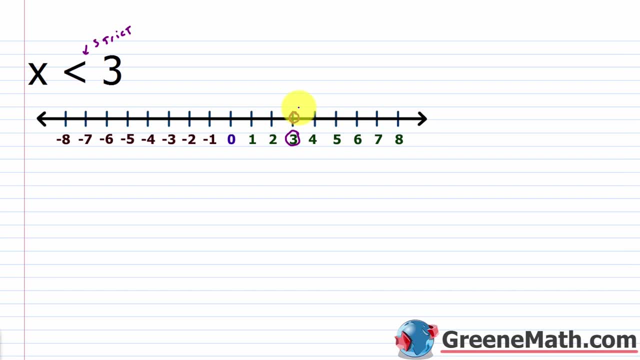 here. So I'm going to put in an open circle or open dot, however you want to think about that, Or more typically, what I use is a parenthesis that faces in the direction of the solution. Here it's a less than So. the solution region is going to the left, So my parenthesis would face: 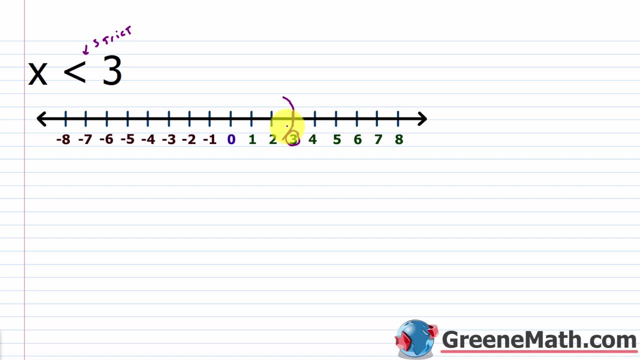 to the left, And I would just shade everything to the left, because all the values to the left of 3 would satisfy this inequality. x is less than 3.. So if I put 2 in there, 2 is less than 3.. That's. 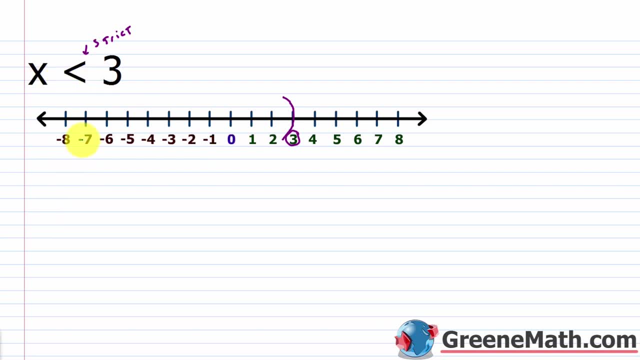 true. If I put 0 in, 0 is less than 3.. That's true. If I put negative 7 in negative, 7 is less than 3.. That's true. So anything to the left of 3 would work as a solution. 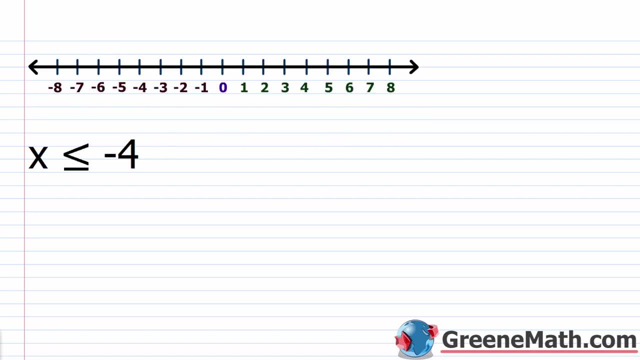 Okay, what about? x is less than or equal to negative 4?? So we want to find negative 4.. So that's right here, And if it's less than or equal to, I've got to include negative 4 as part of my. 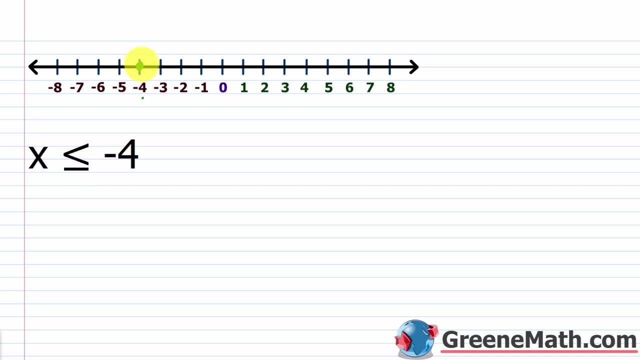 solution. So again, I can put a filled in circle like this, or I can use a bracket. Now the bracket faces to the left because it's a less than or equal to, So put my bracket in there And then I shade everything to the left. 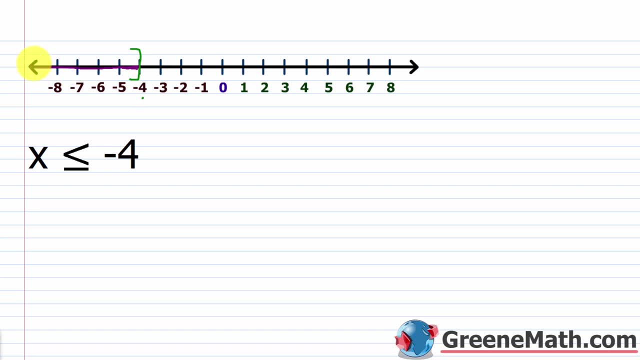 What about? x is greater than 2? I'm going to find 2.. And again, this is a strict inequality, So 2 is not included. I want to put a parenthesis that faces to the right, or an open circle, So I can. 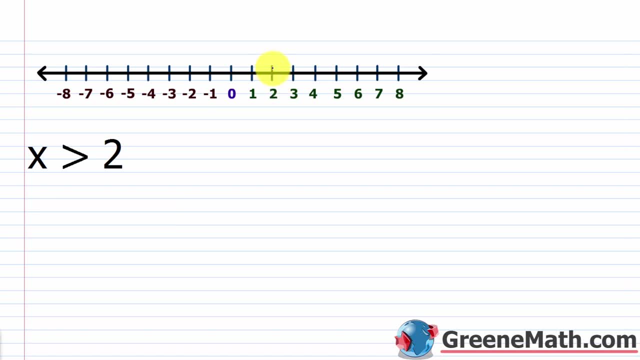 do this or I can do this, And again, it's just a matter of what your textbook or your teacher tells you to do. They both mean the same thing, So let's go with this one for now. So x is greater than 2. So anything to the left of 3 would work as a solution, And again, this is a strict inequality. 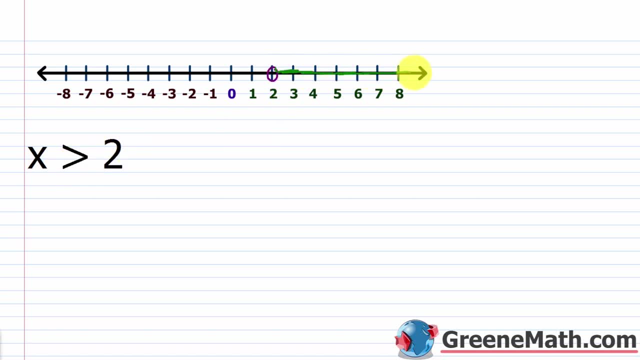 So anything to the right of 2.. So I'm going to shade all this like that And again it's the same thing. if I erase this and I do this, A parenthesis that faces in the direction of the solution region. We have a greater than so. the solution region is to the right. All right. so now that we 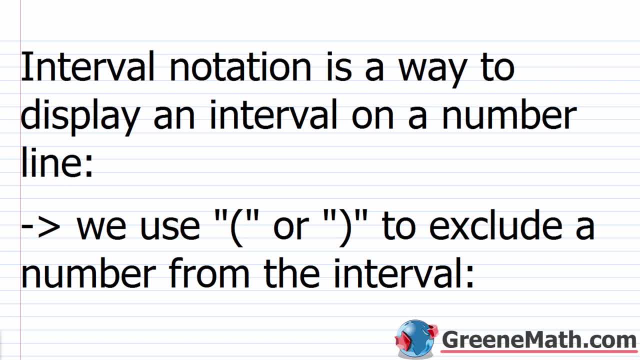 understand how to graph an interval on a number line. let's talk about interval notation. So, as I alluded to earlier, interval notation is a way to display an interval on a number line. Now there's some important things that you need to know here. The first thing is that we use 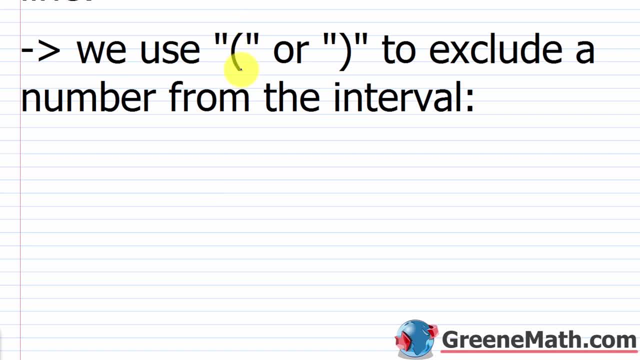 parenthesis. So you have this parenthesis here that's on the left, or this parenthesis here on the right, to exclude a number from the interval. So what exactly does that mean? Well, if I saw something like a parenthesis here and then a value, a, what it's telling me is that it's anything. 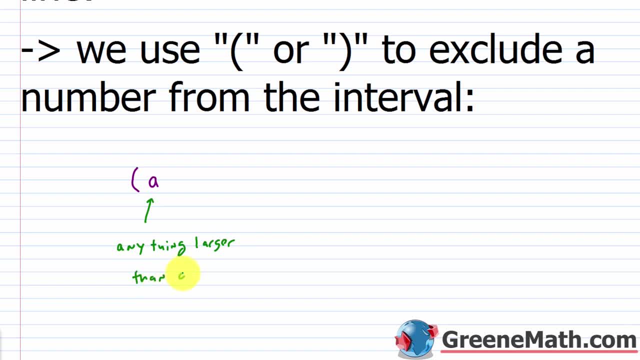 larger than a. A is basically not included. So, for example, if I had x is greater than 2, my interval would start with a- 2 right here, because it's saying anything larger than a- 2.. Can't be 2 itself, but anything larger than 2.. Then you have a comma and let's say I put b there. 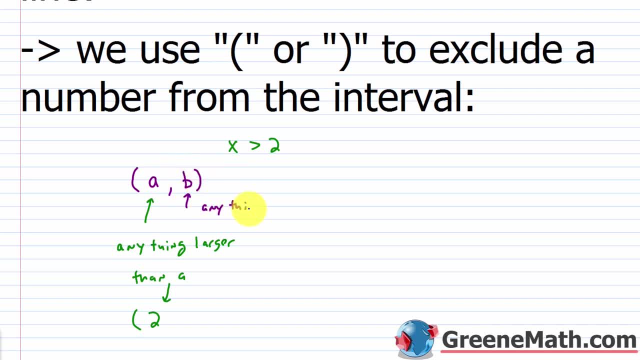 Well, this is anything smaller than b. So in the case of x is greater than 2, well, for this part right here, x can continue after 2, forever and ever and ever. So you use an infinity there, Now, with an infinity because you can't ever touch it. you always use a parenthesis. 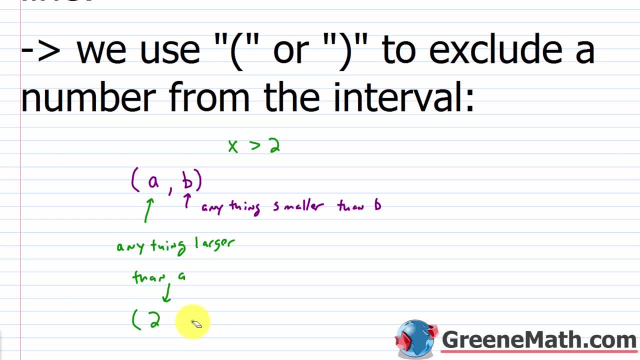 But let's say we had something that was a little bit different. Let's say that we had that x was greater than 2. And x was less than, let's say, 5.. Well, in this case, I want anything smaller than 5, and I also want anything larger than 2.. 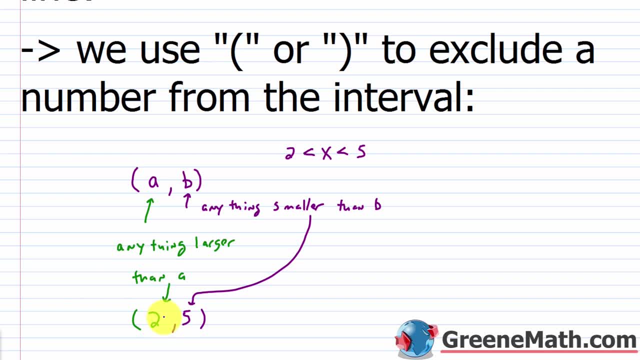 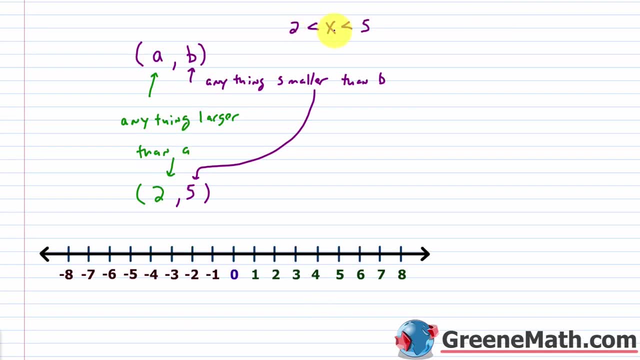 So on a number line that would be the range of values between 2 and 5.. So I have a number line here. If I want to denotate x is greater than 2 and less than 5, I would find 2 on the number line which is here And 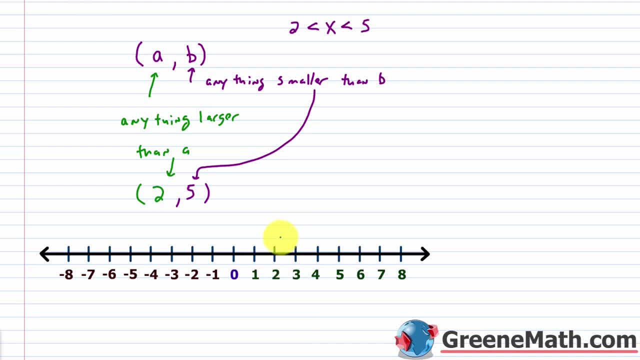 again. we just saw this, So I put a parentheses. That's facing to the right, Because I'm just thinking about x is greater than 2 for right now. So x is greater than 2.. And then now I want to think about x is less than 5.. 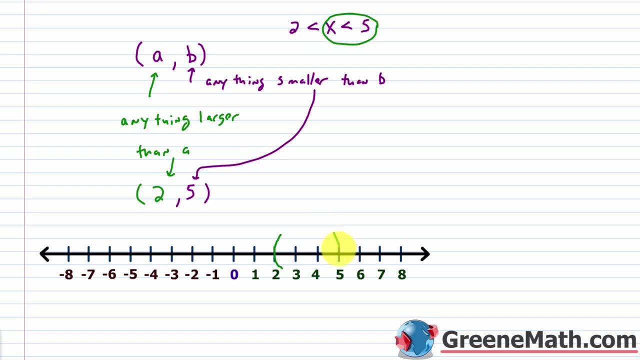 x is less than 5.. So I'm going to put a parenthesis at 5, facing to the left, And I would shade all the values in between, because the values in between are what's going to satisfy this, what we call three-part inequality. 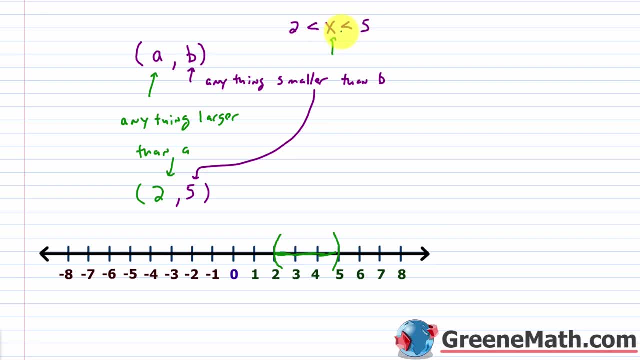 If I have a number that's in between 2 and 5, it works, But if I choose 3,, 3 is greater than 2, and also it's less than 5.. If I choose 4,, 4 is greater than 2, and also it's less than 5.. If I choose something like 6, that's outside of this range. 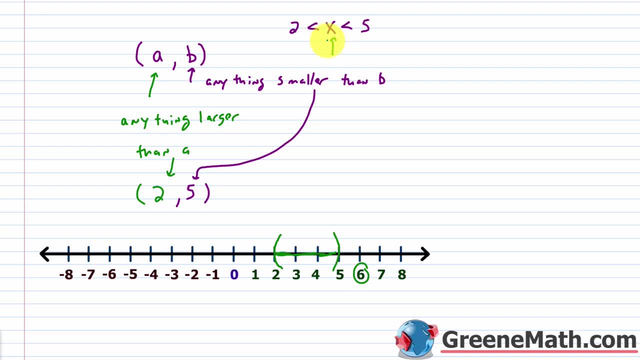 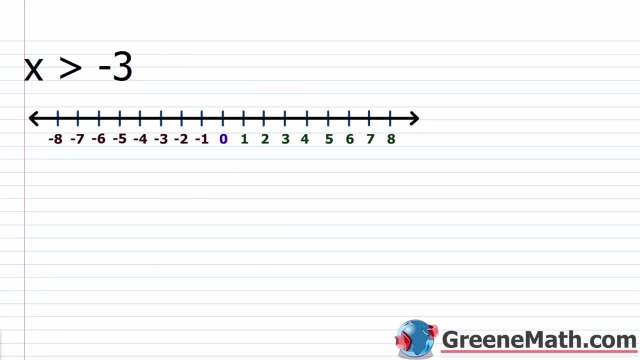 6 is greater than 2, but it's not less than 5.. It's got to satisfy both conditions. So, again, this is how you would notate something like that. So let's look at something like: x is greater than negative 3.. 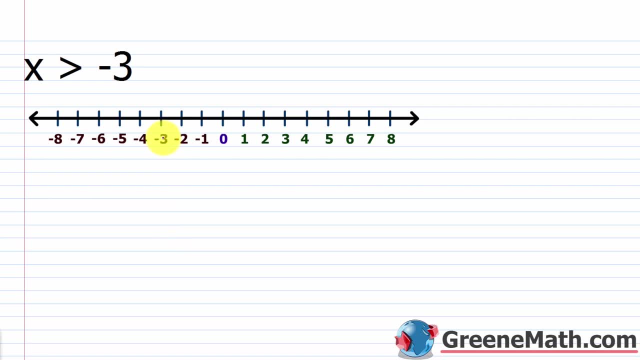 So graphically, we know that we find negative 3. It's greater than So. our parenthesis would face to the right and then I would shade everything to the right here, including this arrow Now in answerable notation. again, it's a strict one. so I know that negative 3 is not included. 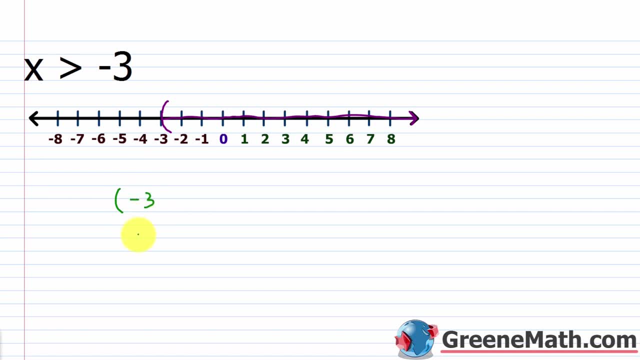 So I have my parenthesis here I put a negative 3. So I'm saying anything or any value larger than negative 3. This is your cutoff point, or your boundary that you're putting in there To say, hey, it's any value larger than this. If I use this exactly, it's not going to work. but anything larger would. 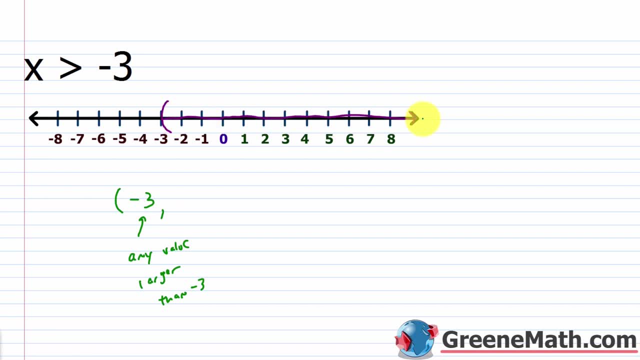 Then comma: This solution continues forever and ever and ever. So the end point: over here we'd put infinity, and we always use a parenthesis with infinity, So I wouldn't say any value less than infinity, because that's, that's not ever going to work. 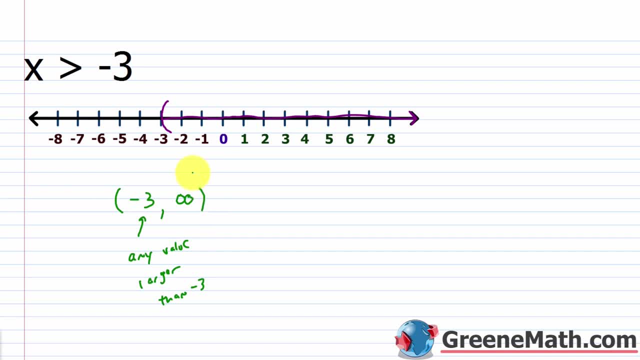 But typically when you have something on this side, we're saying any value, that's less than that. So as another example, let's say I saw- Let's just erase this real quick- Let's say I saw that x was greater than negative 3 and. 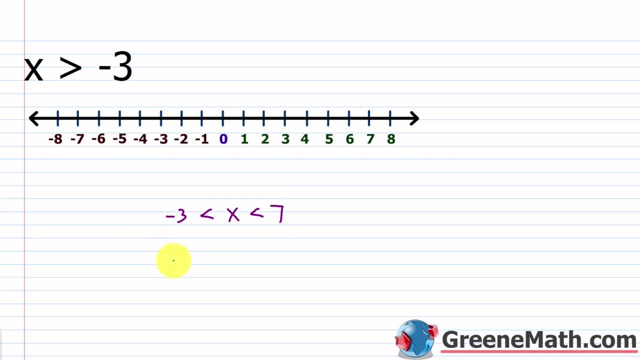 less than, let's say, 7.. Well, in this particular case, in interval notation I'd have a negative 3 next to a parenthesis here: comma: I'd have a 7 next to a parenthesis here. Any value that's larger than this works up to, but not including this value, because it's any value that's smaller than this that works. 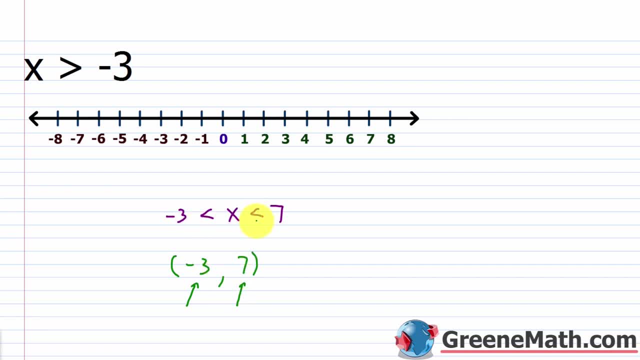 So it's got to be between, between the two values. So if I look at this graphically, at negative 3, I have a parenthesis here. at 7, I have a parenthesis here and I shade everything in between. What about something like x is less than 7?? 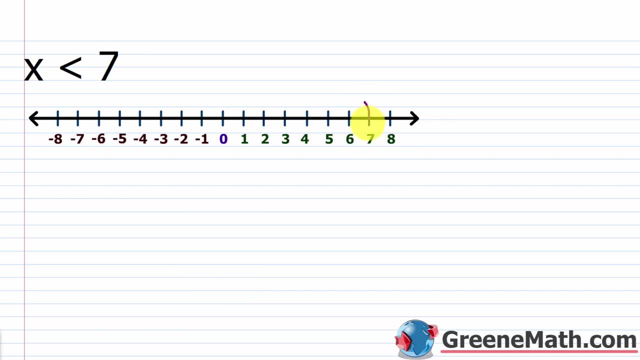 Well, again, graphically, we know, we put a parenthesis that faces to the left at 7, and we shade everything to the left, Pretty simple. And then in interval notation I'll have a 7 here and again. all this is saying is that it's any value? 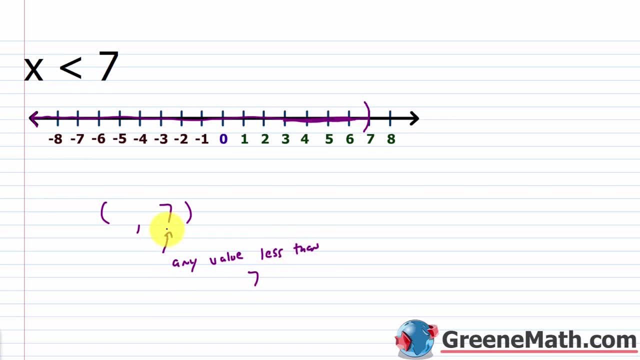 less than 7.. 7 is not included because we have the parenthesis next to it. Now, in terms of going this way, that solution continues forever and ever and ever, It could be anything less than 7.. So it could be negative whatever, however big a number you want to think of. let's say, negative 1 million. 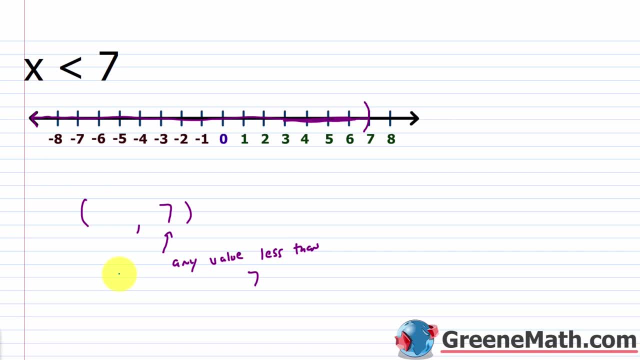 For example, or negative 10 trillion, whatever you want to think of. So we use negative infinity in this particular case. Anytime I use infinity or negative infinity, I always use a parenthesis next to it again, because you can't ever touch it. Infinity is a concept, it's not really a number. 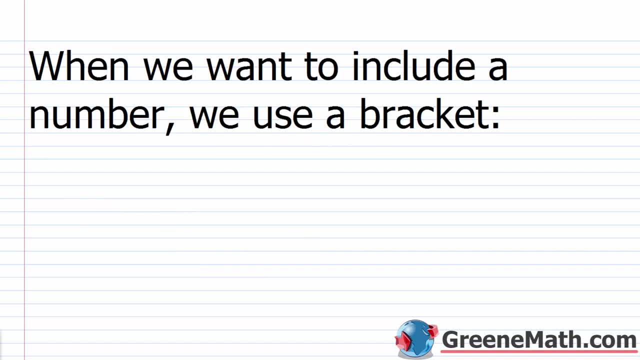 Alright. so in the case that we want to include a number, we use a bracket, just like we did when we were graphing. So something like this means a or larger. So if I had a comma and then infinity that would be, let's say I had. 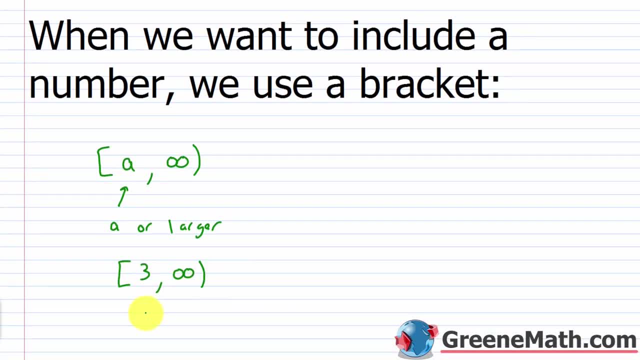 3 with a bracket next to it: comma infinity. This would translate to: x is greater than or equal to 3.. x could be 3 or anything larger. Or let's say, for example, I had a bracket here and I had 7, comma and 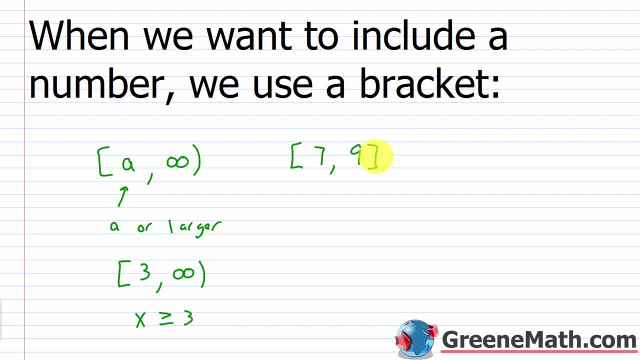 let's say we do 9 in another bracket. This is telling me that x is greater than or equal to 7, and less than or equal to 9.. So it can be 7,, it could be 9, and it could be anything between also. 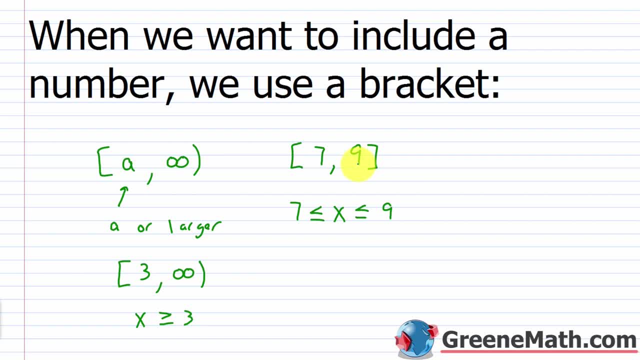 But if you get outside of those ranges, if you go less than 7 or greater than 9, you would not have a true statement. So when we want to again include a number, we use a bracket. So on this part, right here, 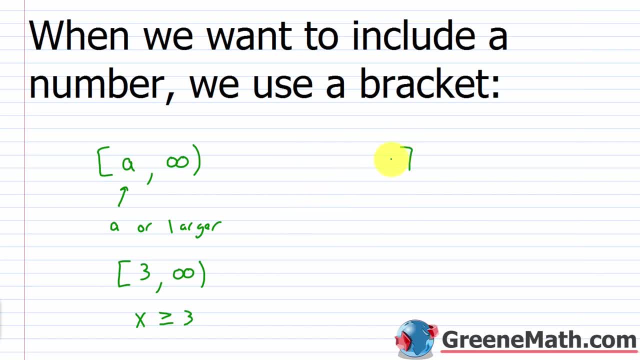 let me kind of erase that. I'm going to erase this On the right side. let's say I have b here, for example. This is b or smaller. Let me put a negative infinity here. So this could be, for example: 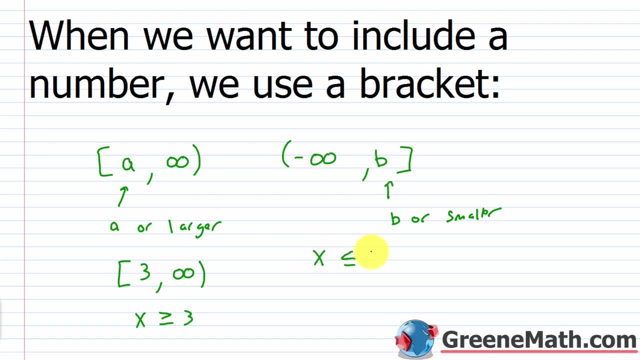 x is less than or equal to, let's say, 10.. Well, in this case it would be negative infinity here, and then up to and including 10, use my bracket. So let's say, as an example, we had 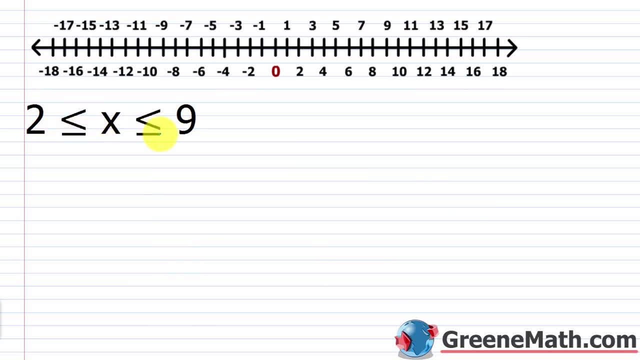 x is greater than or equal to 2 and less than or equal to 9.. So we know that x, again, is greater than or equal to 2.. So let's find 2.. And this number line is a little different because I fit more numbers on it. 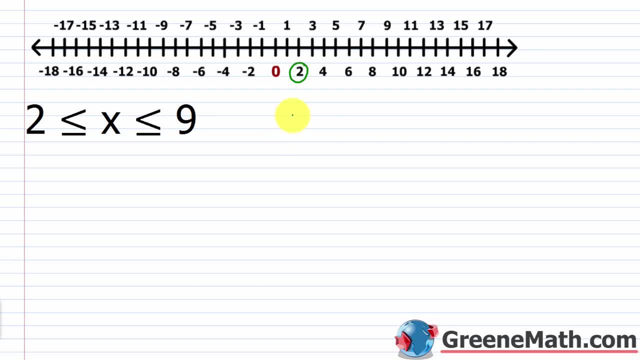 But here's 2 right here, And what I'm going to do is I'm going to put a bracket that faces to the right. I'm going to put a bracket that faces to the right. Now, x is also satisfying the condition that it has to be less than or equal to 9.. 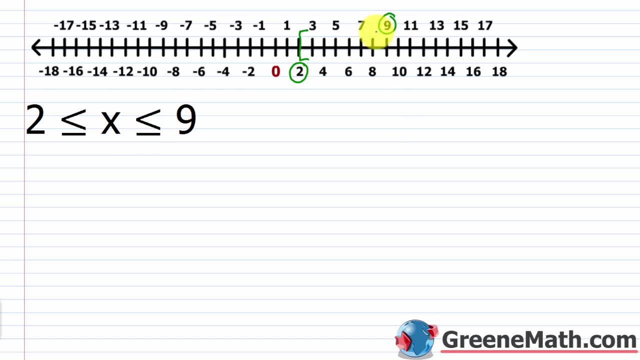 So we're going to find 9, which is right here. Put a bracket that faces to the left And I would shade everything in between there. So x can be 2.. I plug a 2 in there, It's okay. 2 is equal to 2. 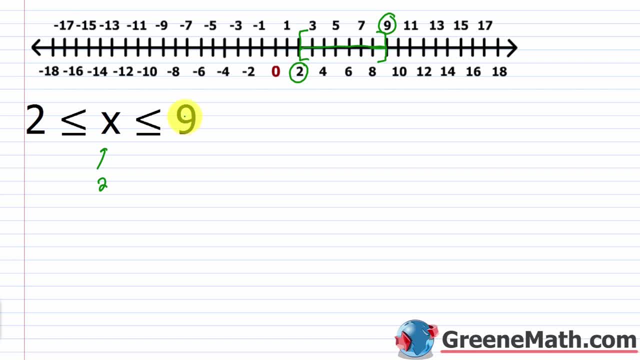 and it's also less than 9.. That works. It could be 9.. Same thing, But it can't be anything outside of this range. If I plug in a negative 3,, for example, negative 3 is not greater than 2,. 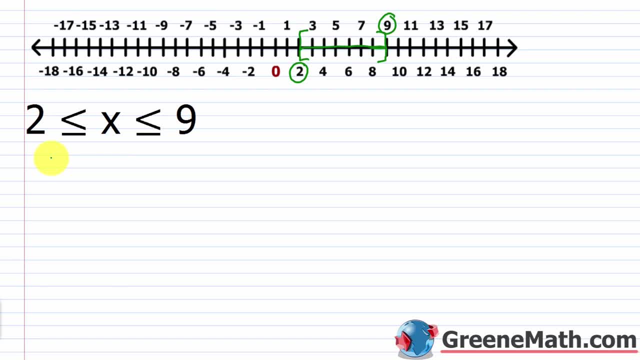 so that would fail. It's got to satisfy both conditions. Now in interval notation I'm just kind of following this right here graphically. I know that the smallest possible value that this thing can take on is 2.. I put a 2 there to the left. 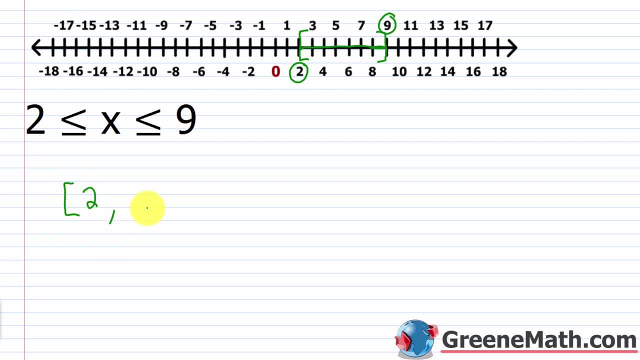 and I have a bracket next to it, Then comma: The largest value this thing can take on is a 9. 9 is included, so I put a bracket there. So this is the smallest value and this is the largest And the only difference. 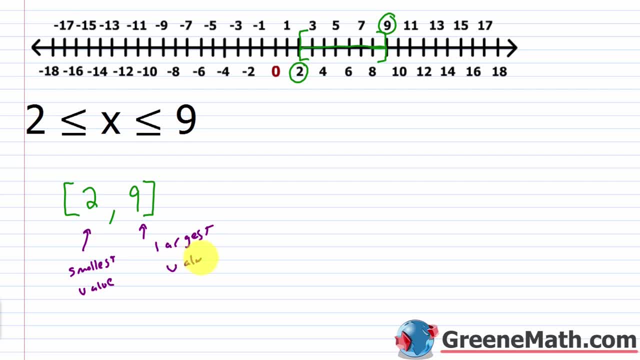 between the two is, let's say I, for example, had x is greater than 2 and also it's less than 9.. What I do in this scenario is I'm basically doing the same thing. I just have parenthesis instead. So I would have a parenthesis there. 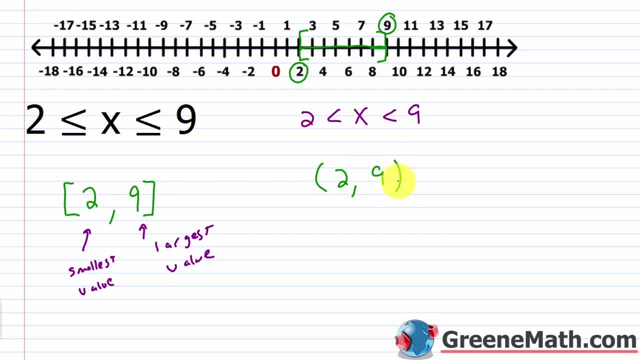 2 comma 9, and then a parenthesis there. In this case I'm saying it's anything larger than 2.. So let's say, hey, it's not 2, but just anything larger than 2.. Then for 9,. 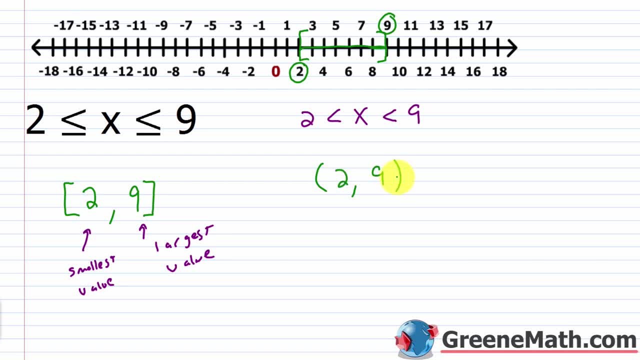 it's not the largest value because it's not included, but it's just anything less than that. So it's between the numbers 2 and 9.. So it's just paying attention to whether you have a non-strict inequality like here or a strict inequality like here. 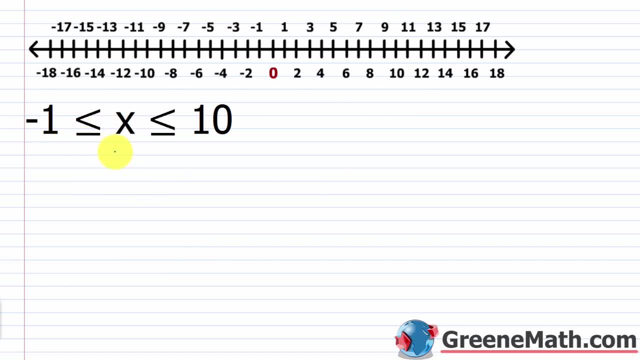 What about something like: x is greater than or equal to negative 1 and less than or equal to 10?? Well, again, graphically pretty simple. I find negative 1.. I put my bracket facing to the right, I put my bracket facing to the left. 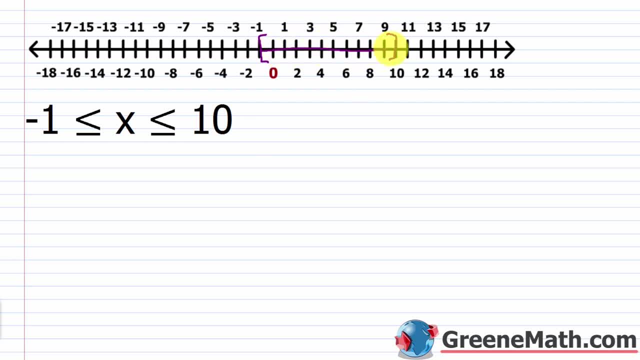 I put my bracket facing to the left and I shade everything between In interval notation. I just basically follow this. I'd have a negative 1 as the smallest value, comma a, 10 as the largest value, and I've got brackets next to each. 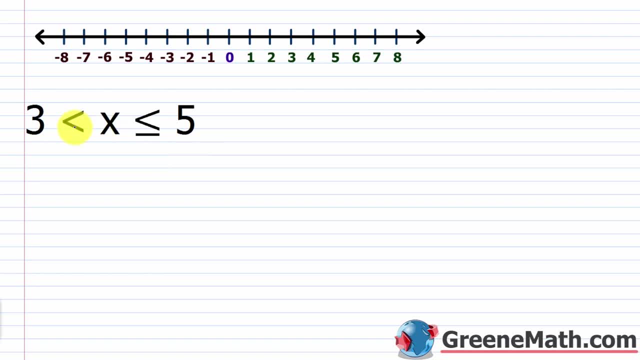 And of course we can have combinations of the two. Here, x is strictly greater than 3 and less than or equal to 5.. So at 3, I'd have a parenthesis that's going to face to the right, Because it's a greater than. 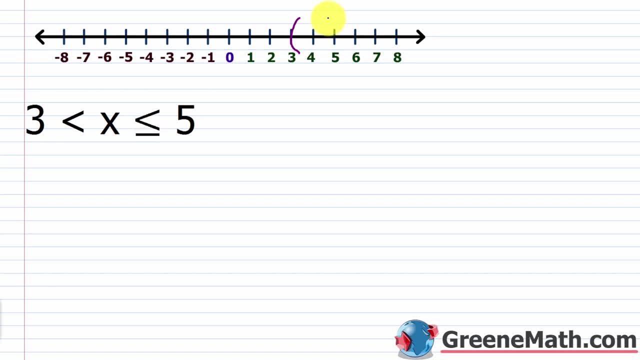 x is greater than 3.. And then at 5, I'm going to have a bracket because it's a less than or equal to 5, so it faces to the left, And I'm going to shade everything in between here And then 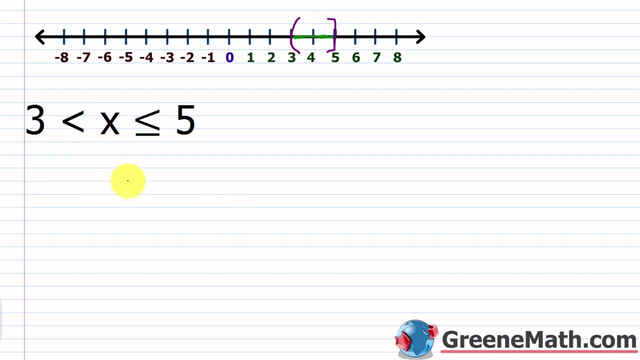 in interval notation. I just follow this. At the left side I'm going to have a parenthesis to say that 3 is not included, Then comma. On the right side I'm going to have a 5 and I'm going to have a bracket. 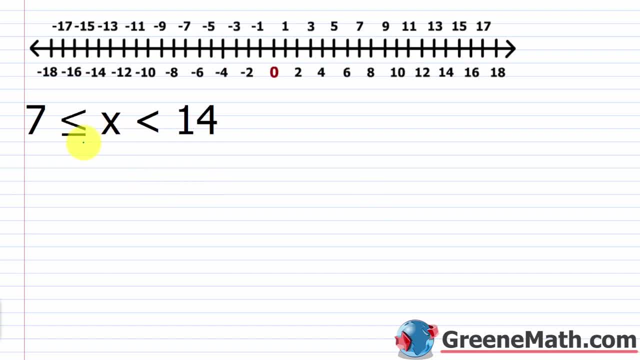 to say 5 is included. Alright, for this one we have that x is greater than or equal to 7 and less than 14.. So if I find 7, I'd want to put a bracket there facing to the right. 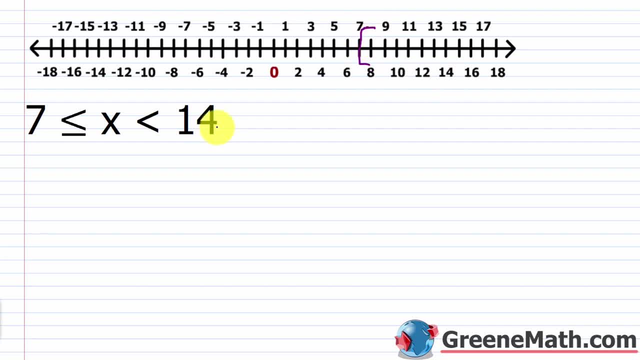 Find 14,. I'd want to put a parenthesis facing to the left And I would shade everything in between In an interval notation. I'm going to have a bracket and then a 7.. Again, 7 is included and then anything. 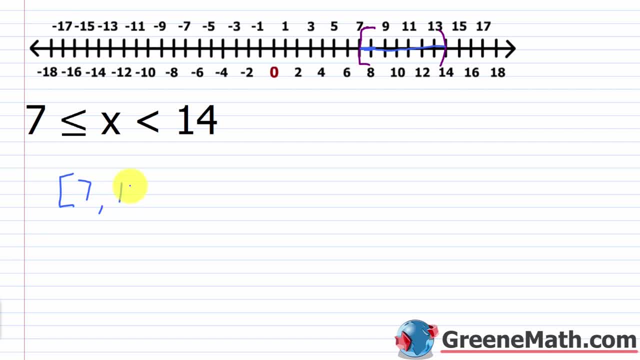 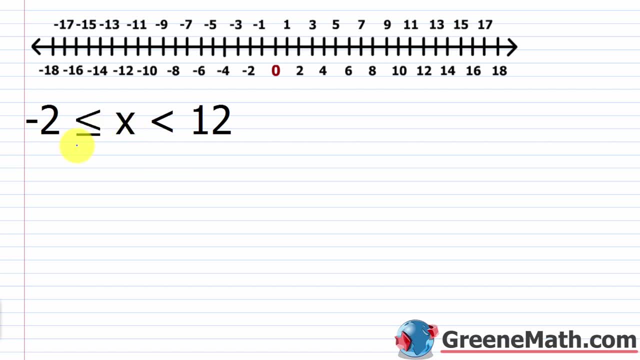 larger up to, but not including 14.. 14 is going to have a parenthesis next to it to say that's not included. What about? x is greater than or equal to negative 2 and less than 12? So here's negative 2.. 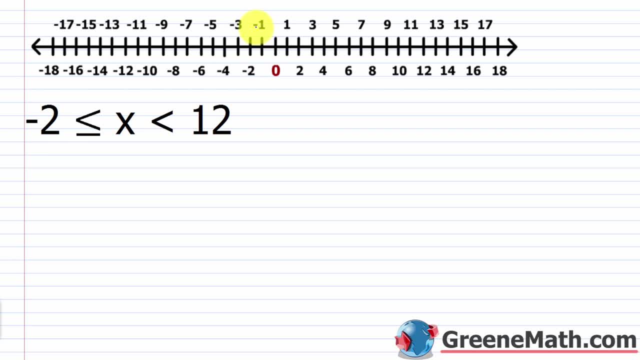 I would have a bracket that faces to the right, And then here's 12. I'd have a parenthesis that faces to the left And I would just shade everything in between And again in an interval notation, I'm going to have a bracket that faces to: 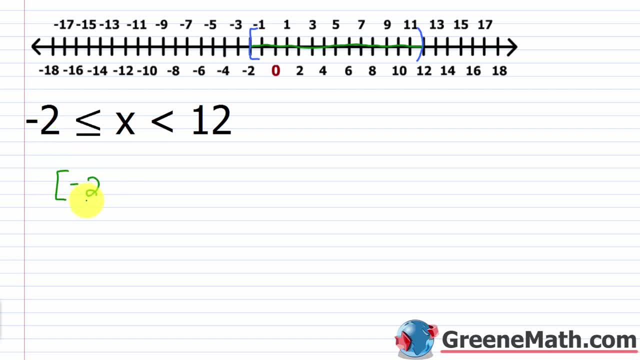 the right, Then negative 2, because negative 2 is included- Comma. and then I'd have a 12. And then 12 is not included. x is strictly less than 12.. So I'd have a parenthesis there to indicate that 12 is not part. 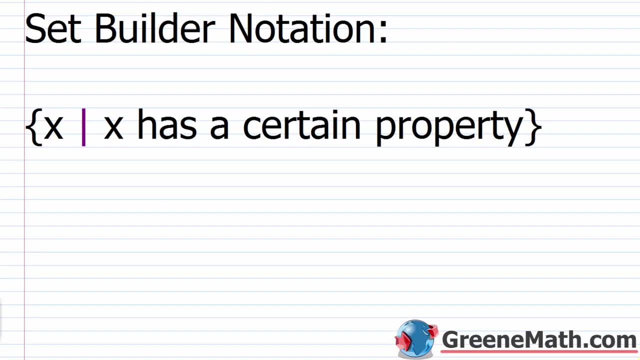 of the solution. So, lastly, I briefly mentioned something known as set builder notation. This is something we will use in math And I didn't really cover it when we talked about sets. So this is a good point where we can kind of 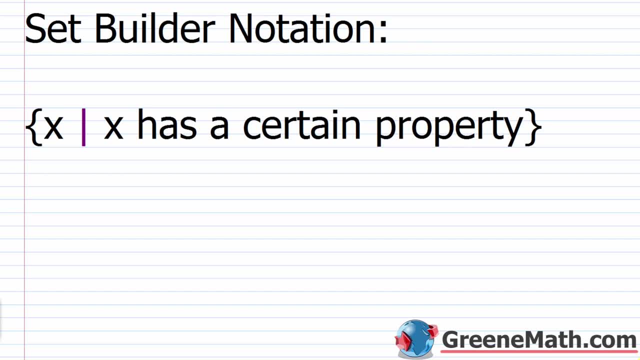 drop it in. So set builder notation. we basically have a variable that's used as a placeholder. This is just saying that it's some real number, And to represent some real number we just use x or y or z, So we say the set of all elements. 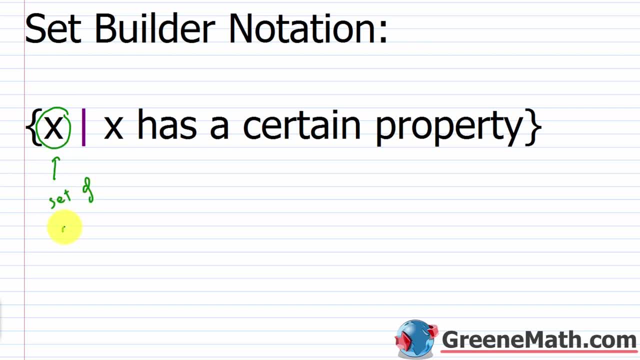 x, The set of all, and this is usually abbreviated by saying the set of all, x, Such that. this bar means such that x has a certain property. So in the example where I have an equation where x is equal to 7,. 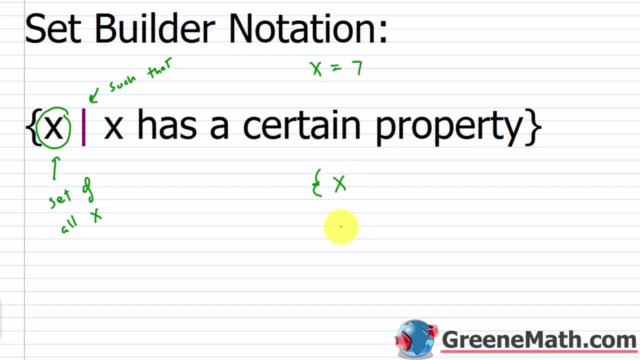 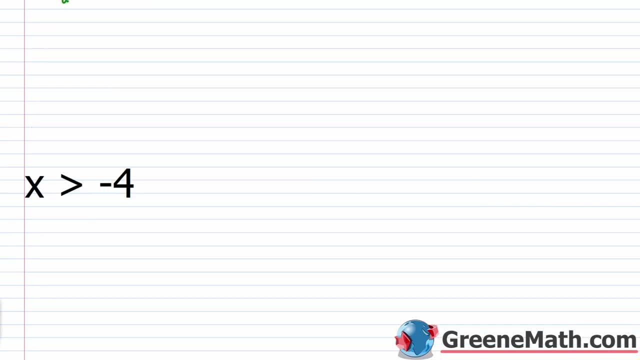 I can notate this by saying the set of all real numbers represented with the variable x, such that x is equal to 7.. Very, very easy. So if I was asked to put something like x is greater than negative 4 in set builder notation. 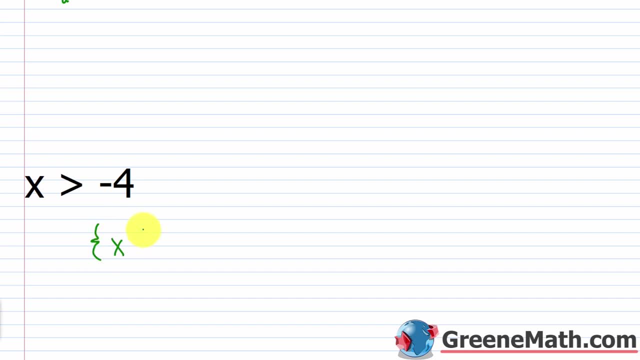 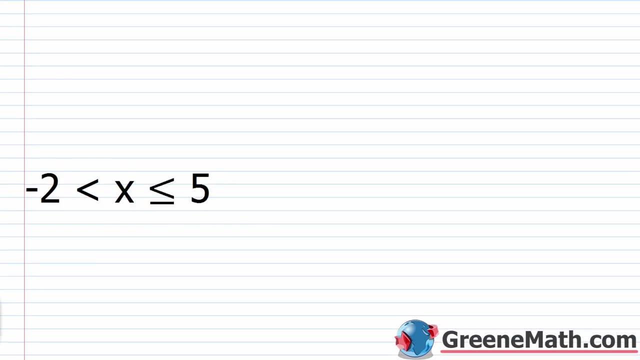 I would say the set of all elements x such that- and then I would just list the property: x is greater than negative 4.. As a final one, let's say we have: x is greater than negative 2 and less than or equal to 5.. 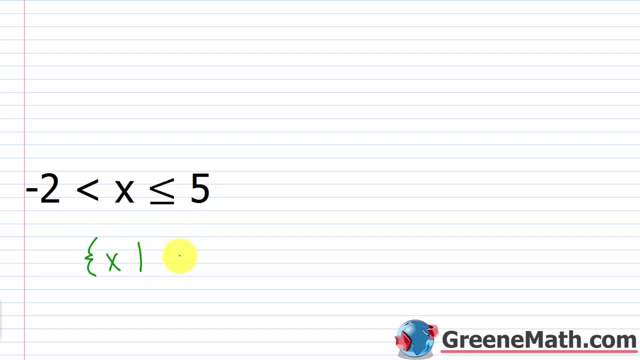 I could say the set of all elements x such that, and then just list the condition: x is greater than negative 2 and less than or equal to 5.. Very, very simple. Hello and welcome to Algebra. 2 Less Than 11.. 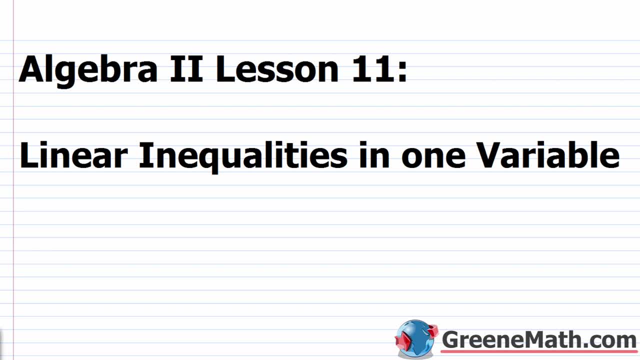 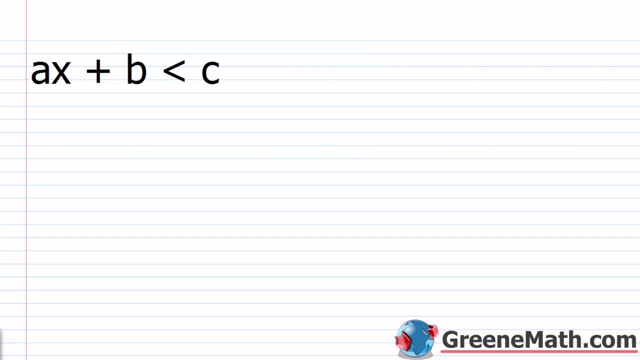 In this video we're going to learn about linear inequalities in one variable. So by the time you get to an Algebra 2 course, hopefully you've had at least some experience with solving a linear inequality in one variable. But even if you haven't, we're going to cover. 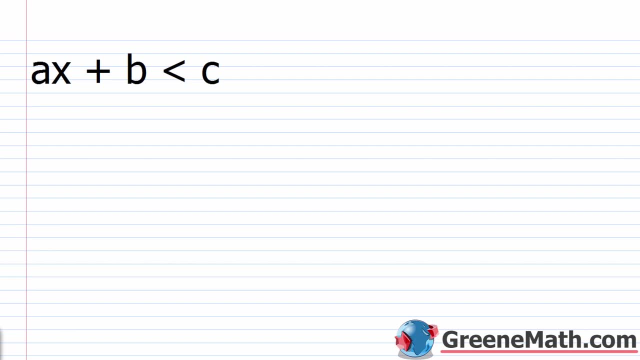 all the details involved with this process and it's going to serve us well in the next lesson and the lessons after that, because we're going to need this as a basis. Now we start off with a generic example where we have ax plus b is less. 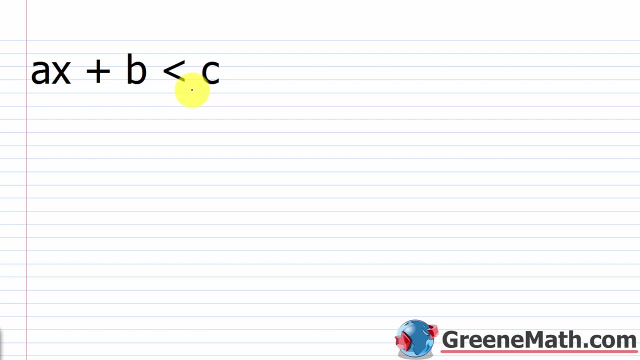 than c. This is something you'd probably see in your textbook, and we can say that a, b and a- c are real numbers. So basically anything you can think of at this point could be plugged in for a, b and c. 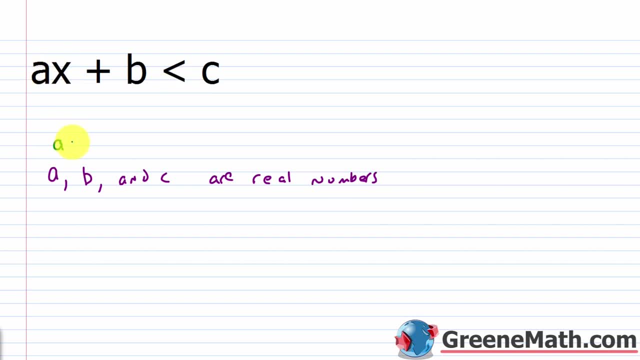 with one exception: a, the coefficient of x is not allowed to be equal to 0. And that's because if I multiply 0 times x, I get 0, and I'd be left with b is less than c. Now there's one other thing. 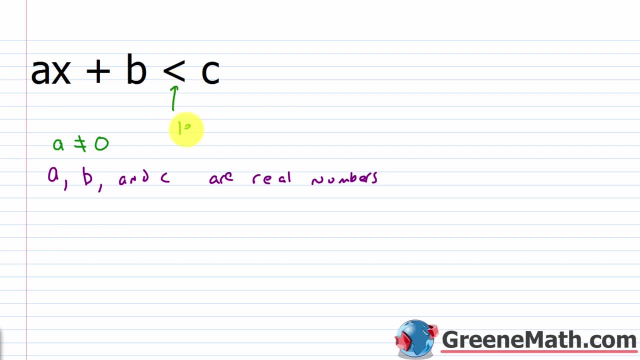 we want to note. We have a less than here. This is a less than. I could replace this with a greater than, or a less than or equal to, or a greater than or equal to. All of those would be equally valid in this generic example. 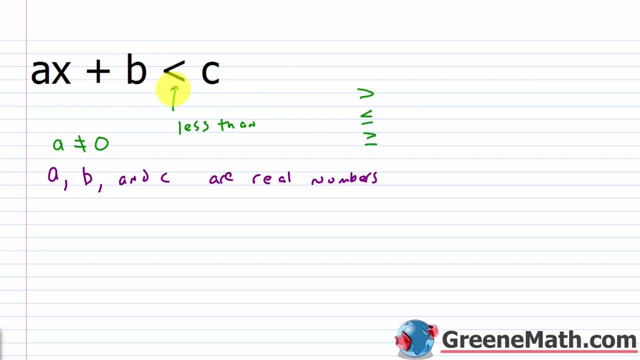 We just have to choose one of them. We just happen to choose a less than So. we have ax plus b is less than c, where again a, b and c are real numbers. a is not allowed to be 0,. 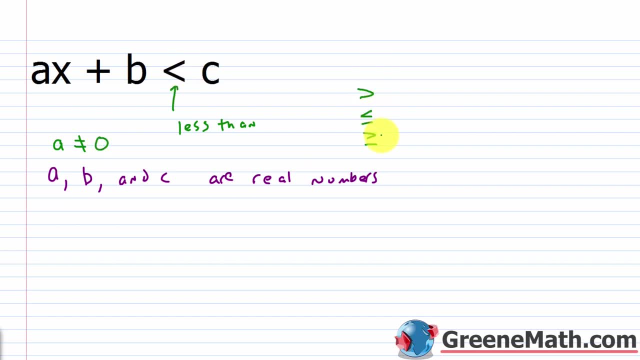 and the less than could be a greater than, a less than or equal to, or a greater than or equal to. So here are just a few examples and we'll get to solving these in a minute. So we have: 2x minus 7 is greater than 5.. 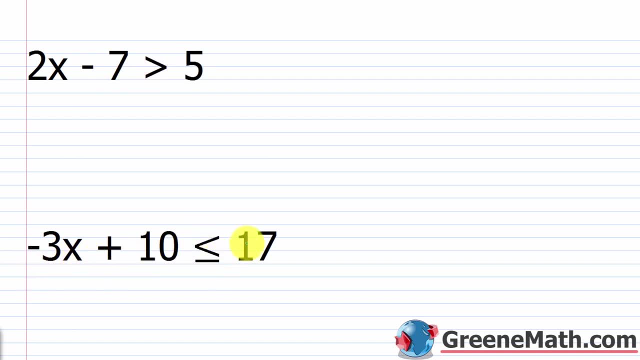 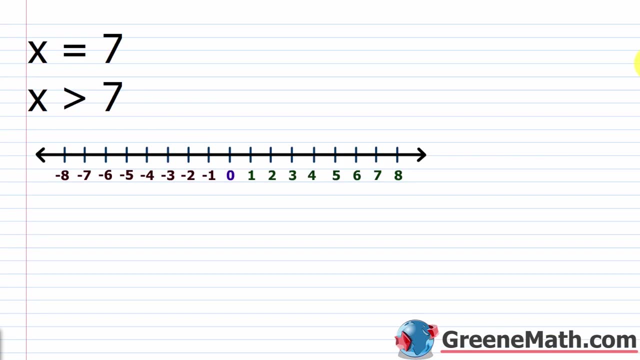 We have negative: 3x plus 10 is less than or equal to 17.. Then we have 0.25x is greater than or equal to negative 2.. So the main difference between an equation and an inequality: with an equation, something like, x equals 7,. 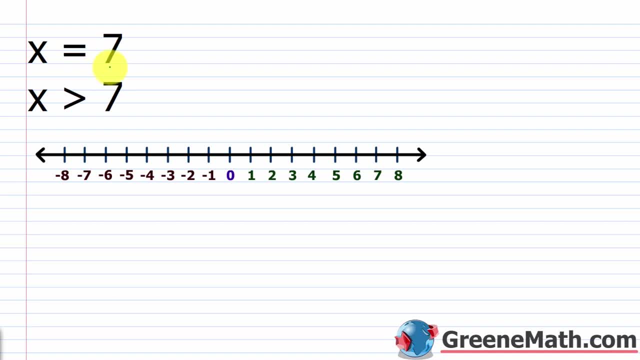 x can be one value there, It can be 7.. It's basically represented with just this. This is: x is equal to 7. With x is greater than 7, if I was to think about that, that's a range of values. 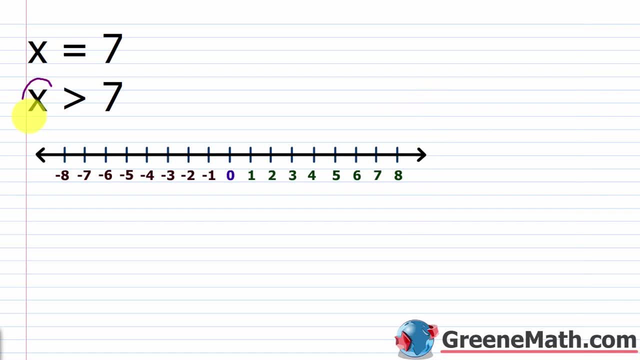 I can plug in anything for x that's larger than 7, and I will get a true statement. I could plug in an 8,, a 9,, a 10,, a 1 million, a 1 billion, As long as it's larger than 7,. 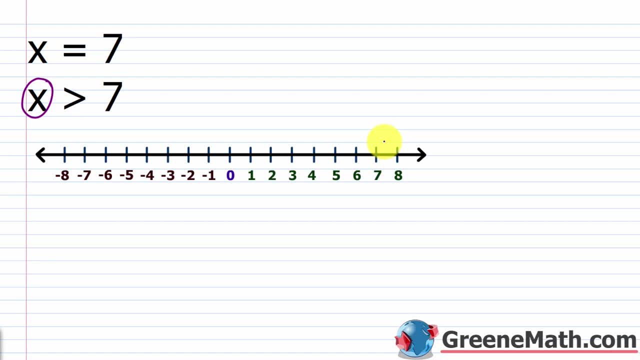 it's good to go Now graphically- and we covered this in the last lesson- at 7, I would put an open source circle or I could put a parenthesis facing to the right. I typically stick with a parenthesis And I would shade everything to the right. 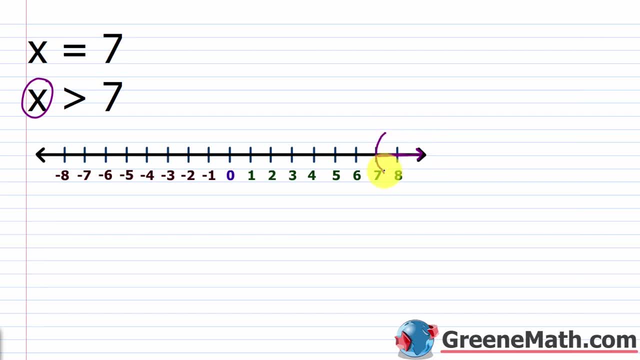 What this means is that 7 is not included in the solution. That's why I have a parenthesis there, Because x is strictly greater than 7.. If I plug the 7 in for x, it wouldn't be true. 7 is not greater than 7.. 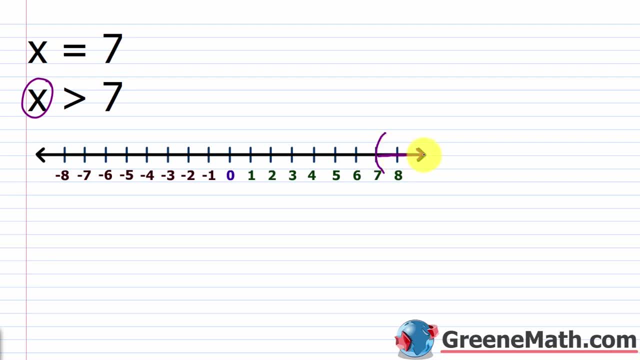 So that's not included. but anything larger than 7,, anything to the right of 7, is. So I shaded everything to the right and I shaded this arrow to say, hey, this is going to continue forever and ever and ever. 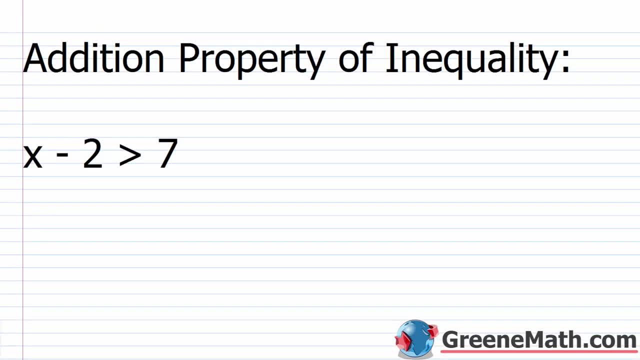 So anything you can pick that's larger than 7 would work as a solution. Alright, so now let's talk a little bit about how we'd solve a linear inequality in one variable, And essentially we use the same techniques as we use when we're solving. 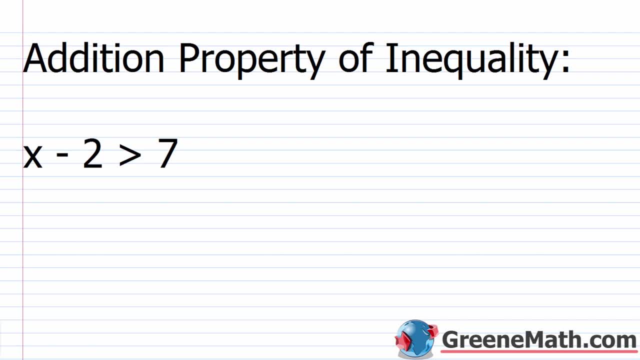 a linear equation in one variable. So you'll recall, when we were solving equations we had this property, known as the addition property of equality. That told us we could add the same value to both sides of the equation and we'd maintain the same solution. 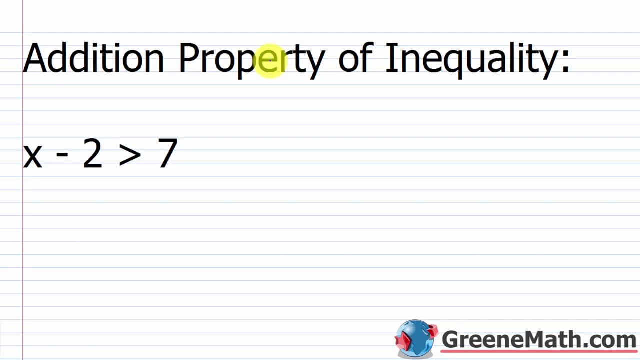 Well, we have a similar property when we work with inequality, So it's called the addition property of inequality, And it's the same thing. It allows us to add the same value to both sides of an inequality. now, and we don't change the solution. 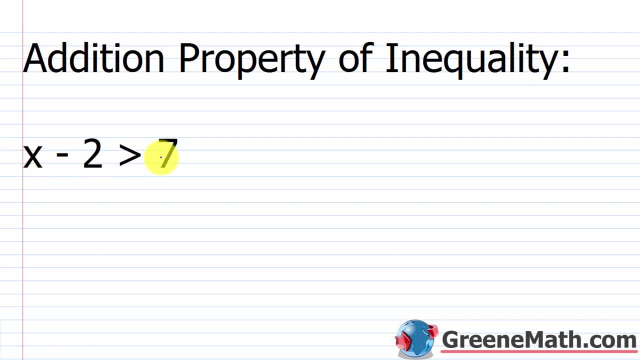 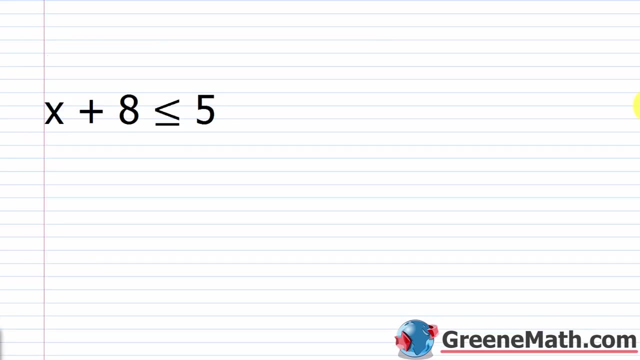 So if I see something like x minus 2 is greater than 7, this is a one-step inequality. So basically, all I need to do to isolate x is just add 2 to both sides of an inequality. This would cancel and you would have x is greater than 9.. 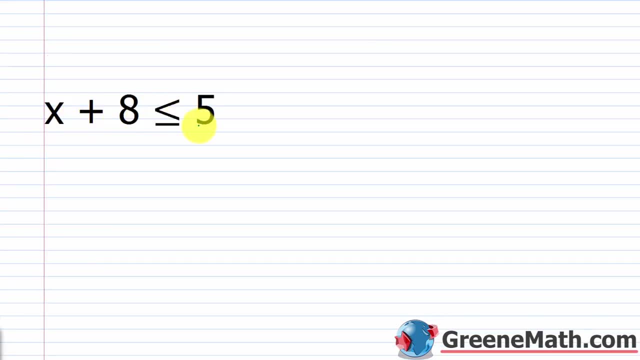 As another example of this, if I have x plus 8 is less than or equal to 5, again, think about isolating x. I just need to subtract 8 away from each side of the inequality, And so this would cancel. 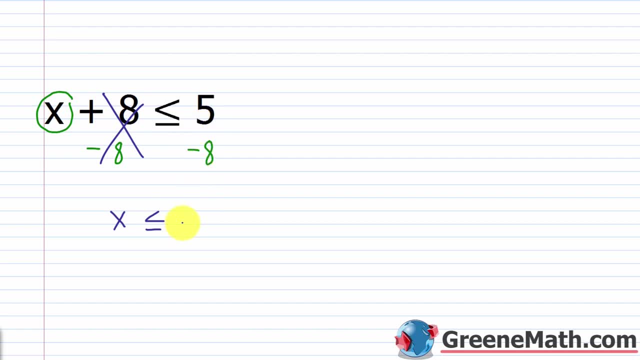 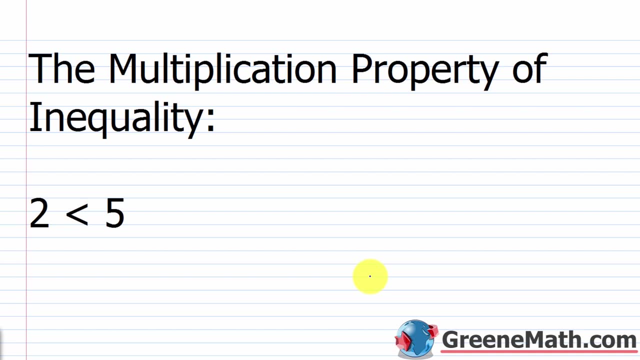 and I would have. x is less than or equal to 5 minus 8 is negative 3.. Alright, for the next property we're going to talk about. it's a little different than its counterpart that is used when we're solving equations. 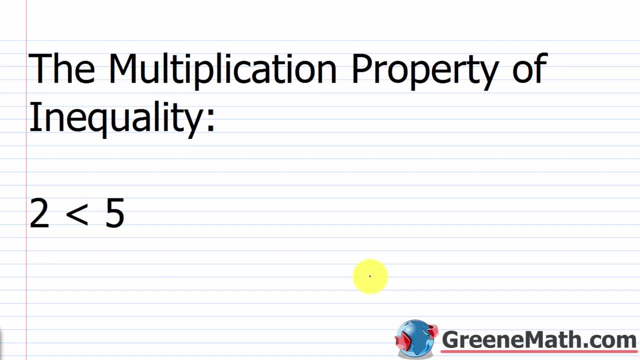 You recall that you have a multiplication property of equality And with this property we can multiply both sides of an equation by the same non-zero value and we will not affect the solution. Well, here, with the multiplication property of inequality, it's different because 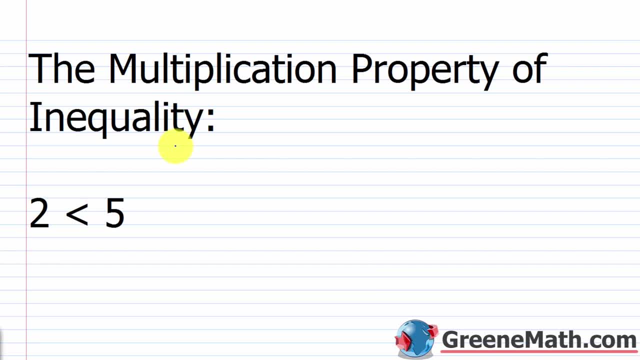 if I multiply both sides of an inequality by the same positive value, it's the same thing. I'll have the same solution. I don't have to do anything. I don't have to worry about anything. you can't use 0 because of the properties of 0.. 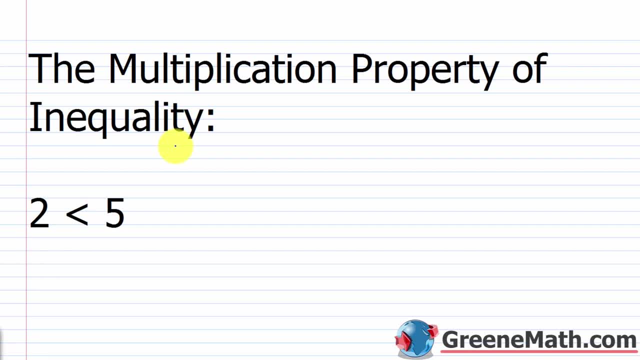 If you multiply by 0, you get 0, so you can't use 0. Anything that's negative, any value that's less than 0, if I multiply both sides by a negative, I've got to flip the direction of the inequality. 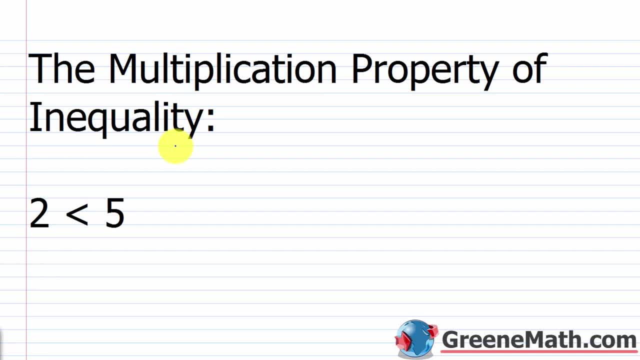 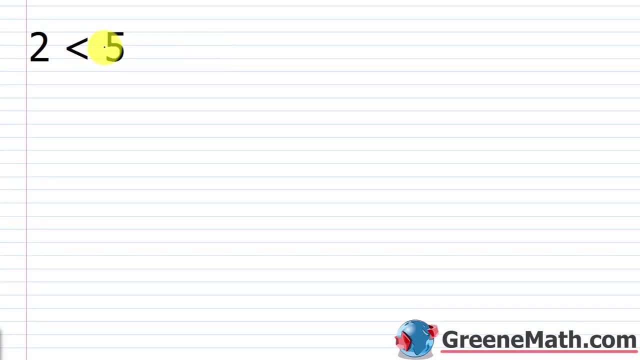 So a less than becomes a greater than, a greater than becomes a less than So, basically, your inequality symbol will flip As an example of why this occurs. if I have, 2 is less than 5, that's true. 2 is a smaller value. 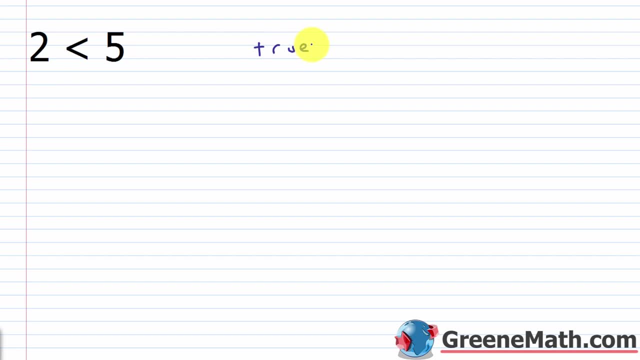 than 5.. If I multiply both sides by a positive, for example, let's say 3.. So 2 times 3 would be 6, and 5 times 3 would be 15.. 6 is still less than 15,. 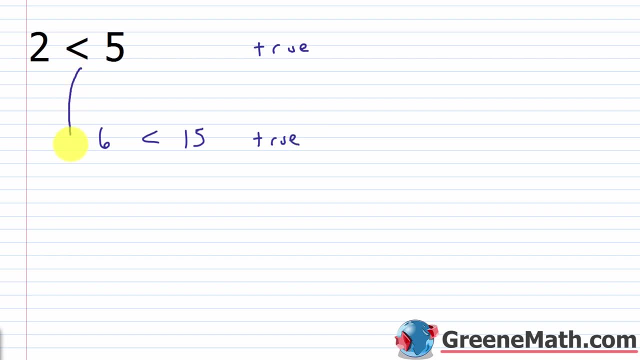 this is true, But if I took this original, 2 is less than 5, and I multiplied both sides by a negative. let's just keep it simple and say negative 1.. What's going to happen is I'll have negative 2. 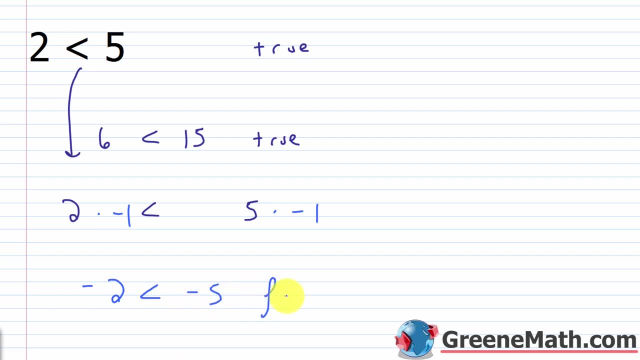 is less than negative 5.. This is now false. Why is it false? Because I started out with a bigger number here. when I applied a negative to it, it became a bigger negative. Negative 5 is a bigger negative than negative 2.. 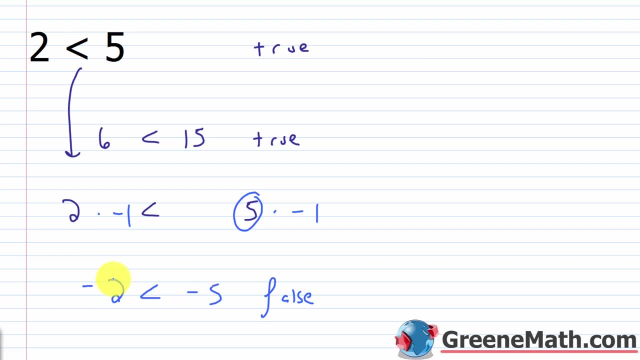 A bigger negative is actually a smaller value. You think about the way a number line works. a bigger negative is to the left And as we go to the left numbers actually get smaller And it's a hard concept to kind of wrap your head around. 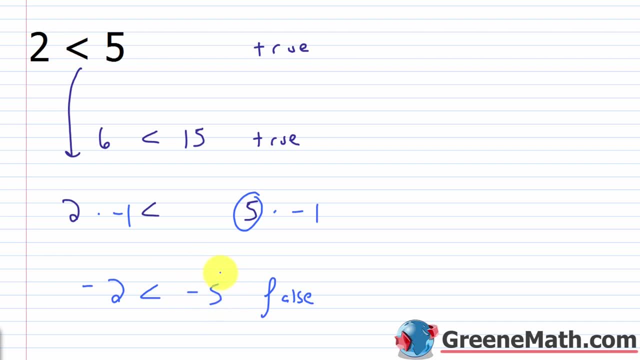 because, generally speaking, until we get into algebra, we think of the number 5 as being larger than 2.. So that kind of sticks with us for a while until we can shake free of it. So negative 5 is a smaller value than negative 2.. 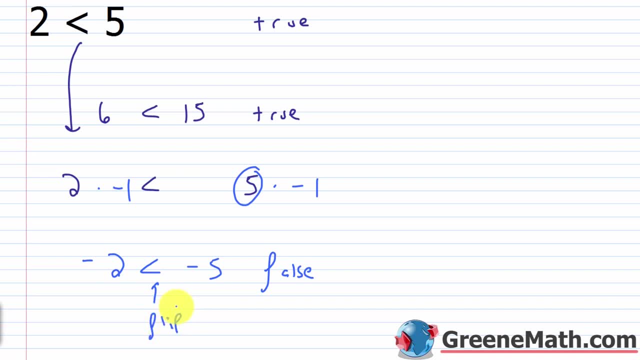 So for this we need to flip it. So we're going to flip, and so if I change the direction of the inequality meaning I go from a less than to a greater than, this now becomes true: Negative 2 is greater than. 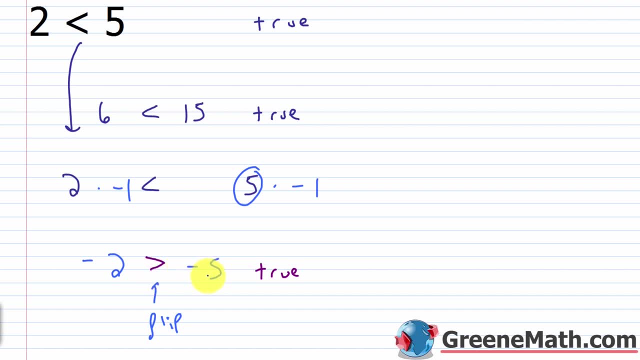 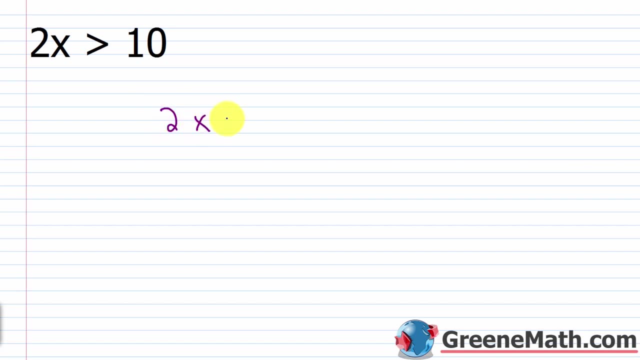 or is a larger value than negative 5.. Alright, so let's look at an example here. We have: 2x is greater than 10.. So we know if we had: 2x is equal to 10, we divide both sides of the equation by 2,. 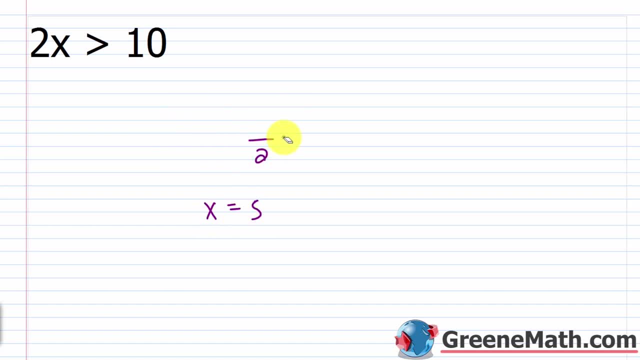 we get x equals 5.. It's the same thing here. I want to isolate x, and so I want to divide both sides of the inequality by 2. so that I can do that, I get x is greater than 5.. Because I divided both sides. 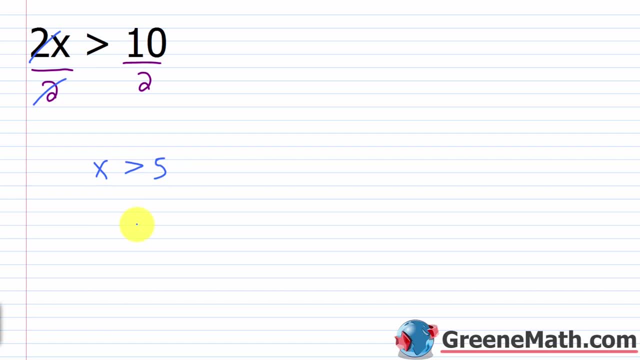 by a positive, I didn't have to flip the direction of the inequality symbol. If I would have had a situation where it was, let's say, negative 2x is greater than 10, well, in this scenario, I divide both sides by a negative 2,. 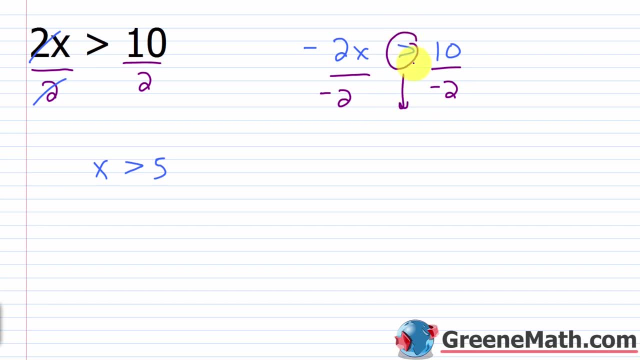 I've got to flip the direction of the inequality. Right now it's a greater than, it's going to become a less than, So it's the symbol flips. So this becomes a less than, and this will become: x is less than negative 5.. 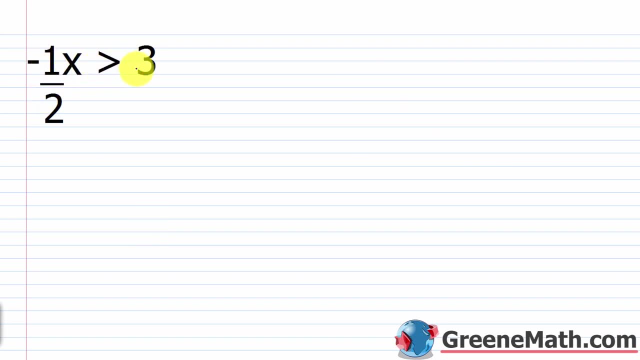 Alright, let's say we saw something like negative 1 half x is greater than 3.. What would I do to isolate x? So negative 1 half x is greater than 3.. Well, I want to get x by itself and what I can do is: 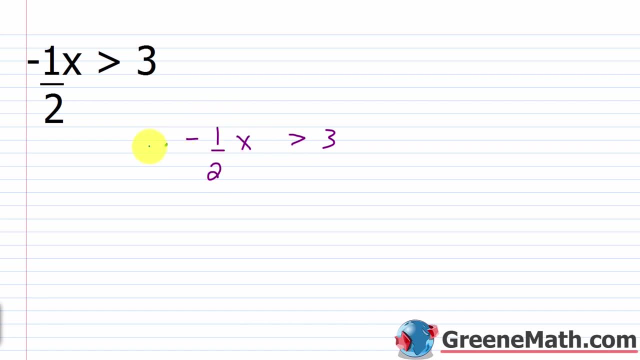 I can multiply both sides of the inequality by the reciprocal of this, so that's negative 2 over 1, or basically negative 2.. And so this is going to cancel with this. but what I've got to remember again because I multiplied by a negative, 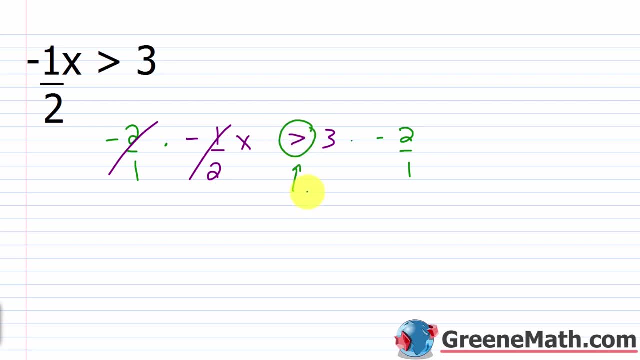 and I'm working with an inequality. I've got to flip the direction of the inequality. It's a greater than so, it's got to become a less than So. the symbol there again, it's a greater than, it's going to become a less than. 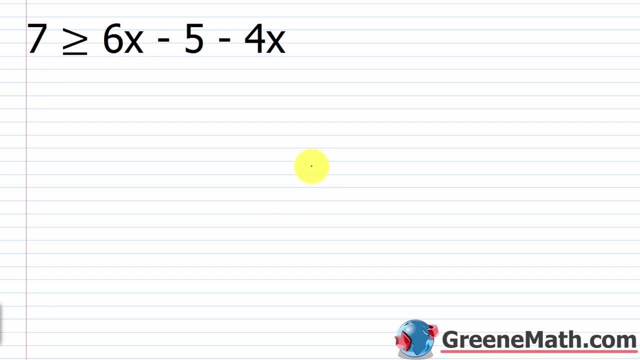 So this is x is less than. it's time to look at some sample problems. So we have that 7 is greater than or equal to. we have 6x minus 5 minus 4x. So just like with an equation. 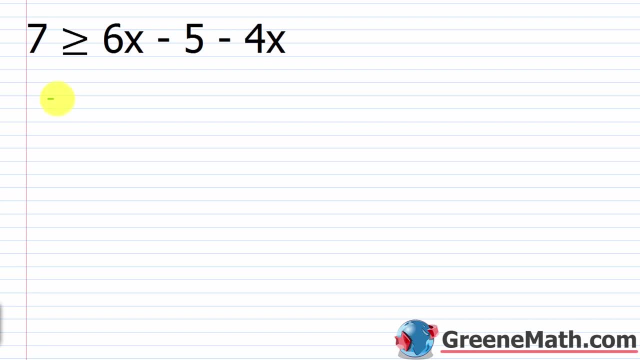 I'm going to simplify each side first. So I have: 7 is greater than or equal to. we have 6x minus 4x, that's 2x, and then minus 5.. Make this a little cleaner. So now I want the variable term. 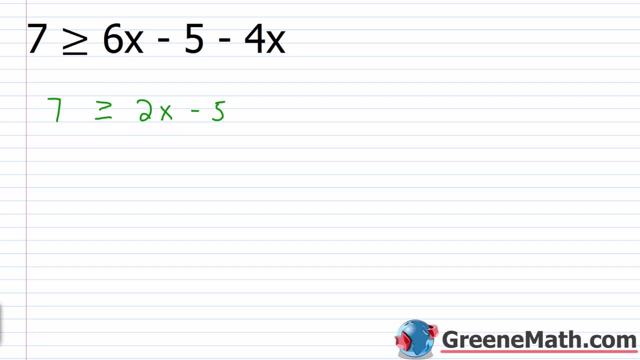 on one side of the inequality, the number on the other. So I can simply add 5 to each side of the inequality. 7 plus 5 is 12.. So 12 is greater than or equal to. we have 2x. 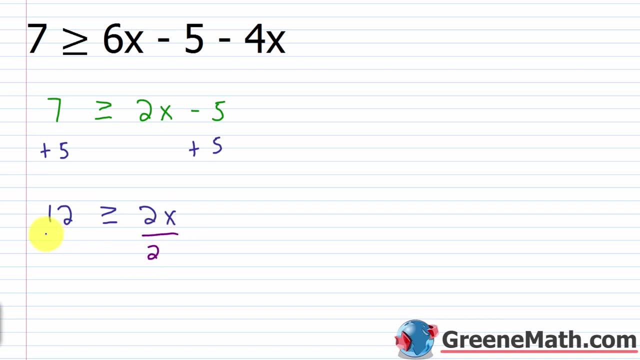 To get x by itself, I would divide both sides by 2.. Now that's a positive number, so I don't need to do anything to the inequality symbol. This cancels with this and gives me 6. So that's greater than or equal to. 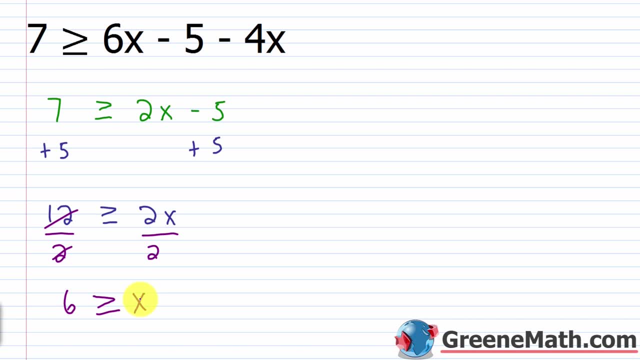 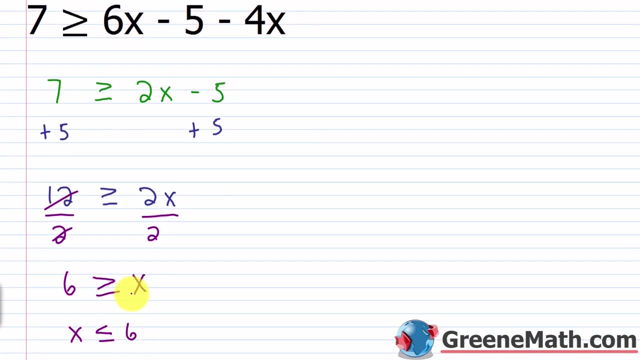 and then we have x. Now, typically, I like the variable to be on the left And using interval notation, So to flip it. if your symbol is pointing to x, that means x is less than or equal to 6.. These are the same. 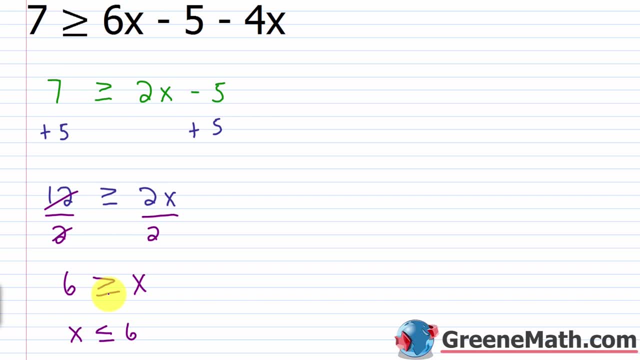 6 is greater than or equal to x, or x is less than or equal to 6.. It's just easier to read this because typically we read from left to right. There's two things I want to show you real quick. In our last lesson we showed 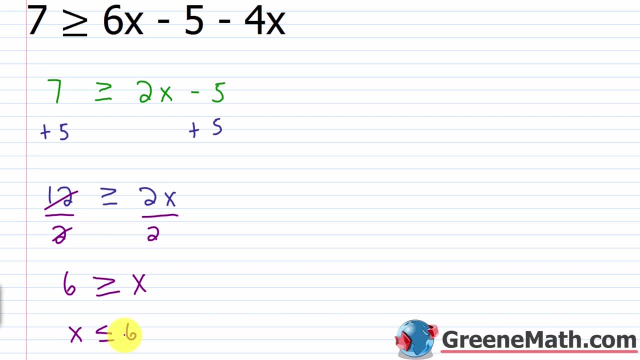 how to write something in interval notation and we showed how to graph an interval on the number line. But I missed that lesson and that's fine, Because I'm going to show you really quickly how to notate this solution. So the first thing with interval notation is: 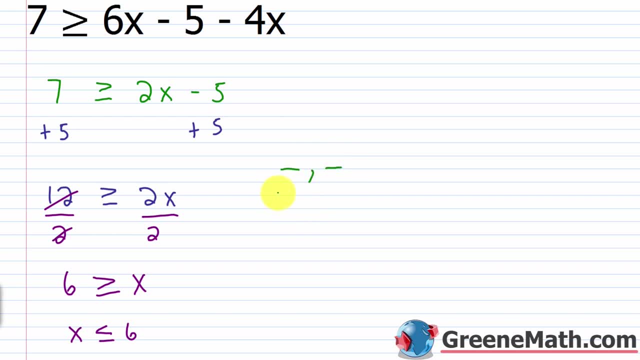 you have basically a value here, a comma and a value here. So this right here we think of as the smallest and this right here we think of as the largest. So, when we think about, x is less than or equal to 6,. 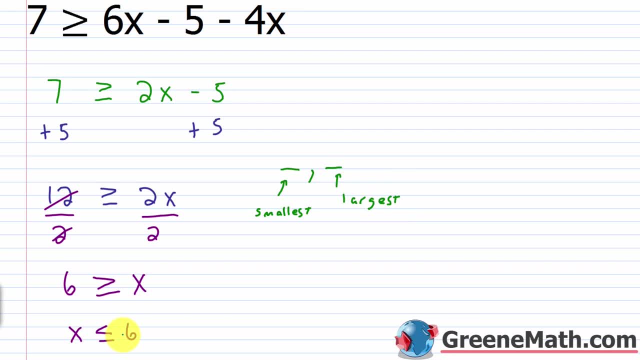 what is the smallest value that x can take on? It's going to be 1.. Because x is less than or equal to, so any value less than 6 that you can think of is going to work. And that goes on forever and ever, and ever. 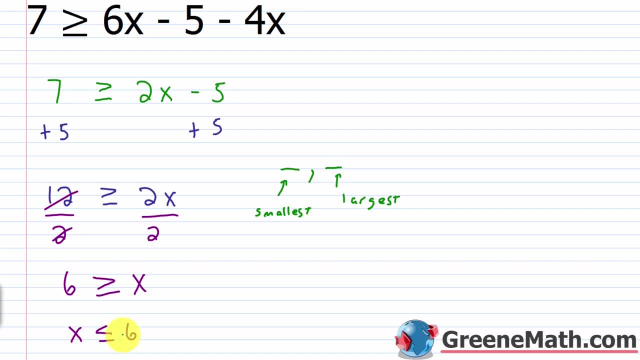 I could do negative 1 trillion. That would work. So, to show this, we use infinity And specifically there, because it's in the negative direction, we use negative infinity. Now, when I use negative infinity or positive infinity, what I place next to this is a parenthesis. 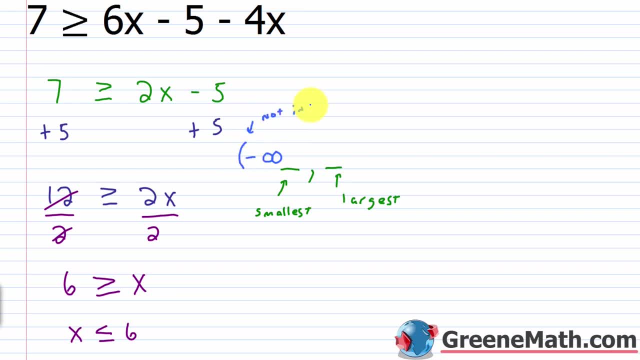 The parenthesis says not included. So the smallest value doesn't exist. so we use negative infinity. Now for the largest possible value. we know it's 6.. x can go up 2 and include 6. So I put a 6 there. 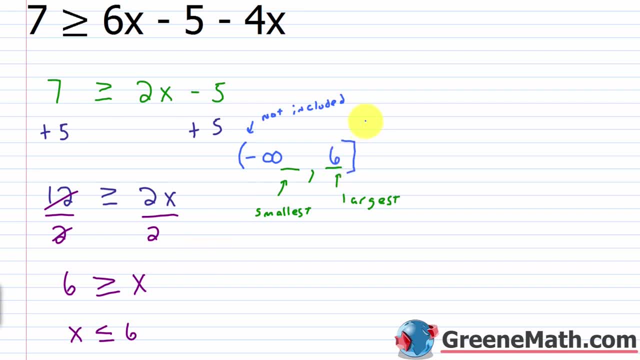 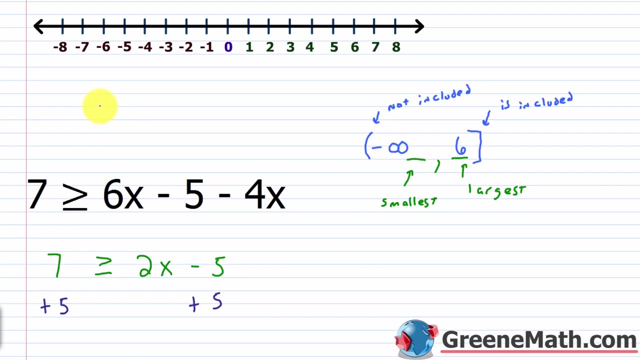 and then, because 6 is included, I use a bracket. This means is included. So 6 is the largest value and it's included, so we use a bracket. Now, graphically, it basically looks like this. Let's go up to a graph. 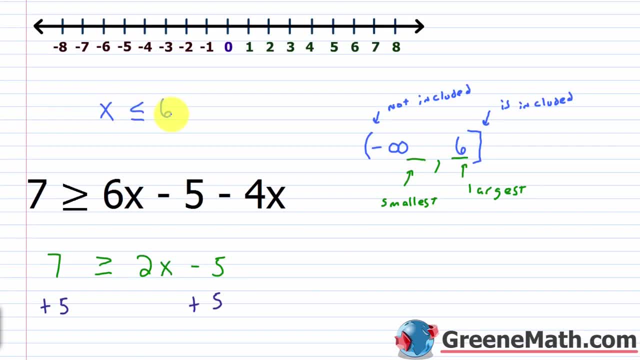 Let me write my solution here. It's x is less than or equal to 6.. So on a number line I would find 6,, which is right here, And I can put either a filled in circle like this or I can use a bracket. 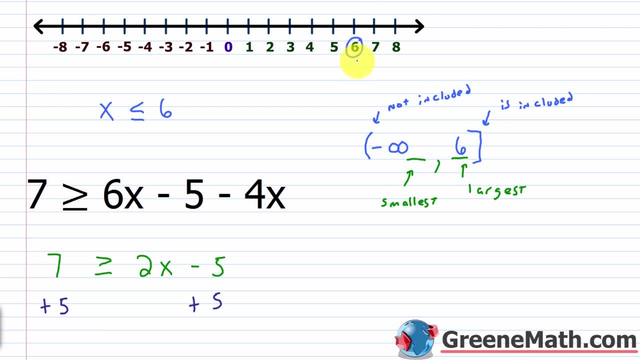 that faces towards the solution region. The solution region is going to the left because we have a less than- Let me make that a little better- And I want to shade everything to the left. So all these values that satisfy that inequality And I can't list. 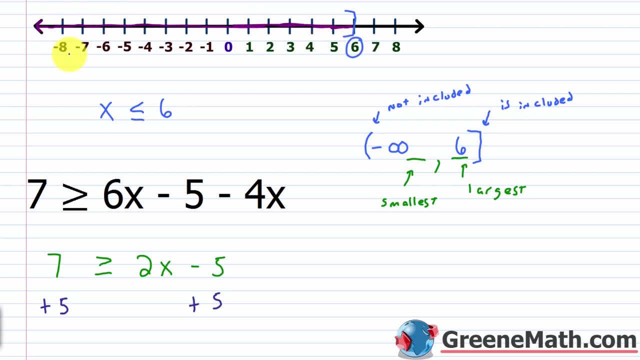 all of them. so I'm going to shade that arrow to say the solution continues forever and ever and ever. Now, looking at the graph and looking at interval notation, you can see some similarities. We use a bracket at 6.. We use the bracket at 6.. 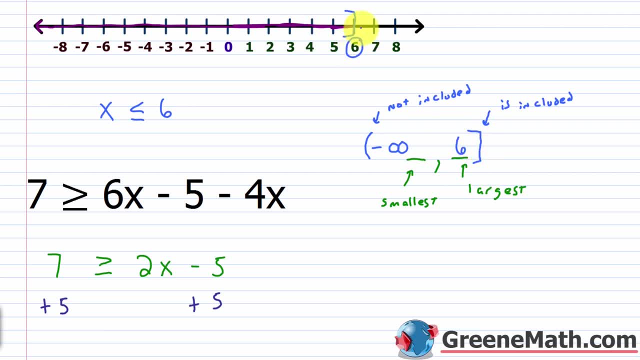 Again, that tells us that 6 is part of the solution. And then it continues forever and ever and ever. We have this arrow here that's highlighted. You can kind of think about this being that. That arrow tells us it continues forever and ever and ever. 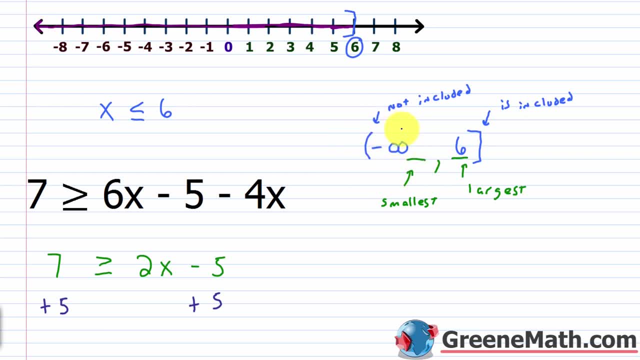 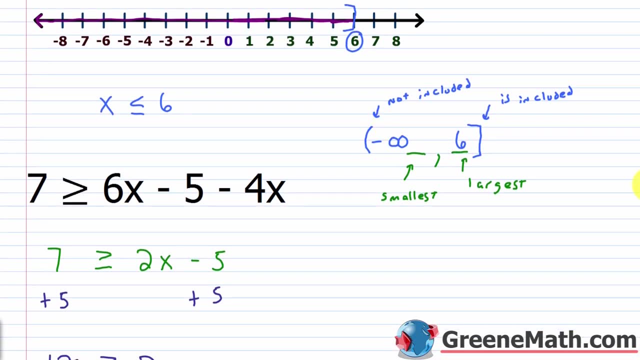 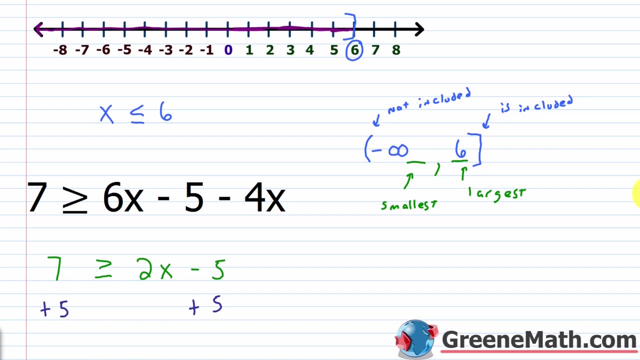 In interval notation we express this by saying negative infinity is in place of the smallest value, because we don't really have a smallest value. So before we kind of move on, you know, in Algebra 1 I checked almost everything. In Algebra 2, I'm not checking as much stuff- 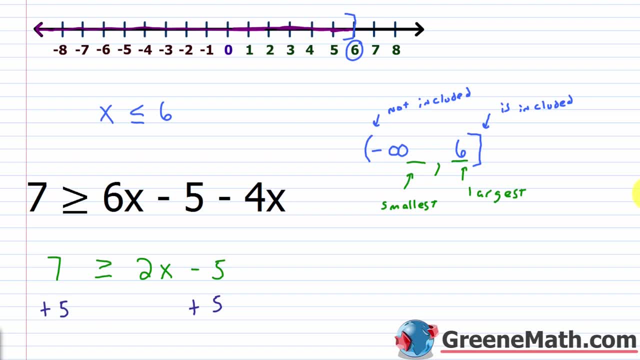 just so we can get more in. But I want you to know how you can go about checking your answer for this. It's a lot more tedious than checking an equation. The first thing is you would replace your inequality symbol with equals. So let me erase this real quick. 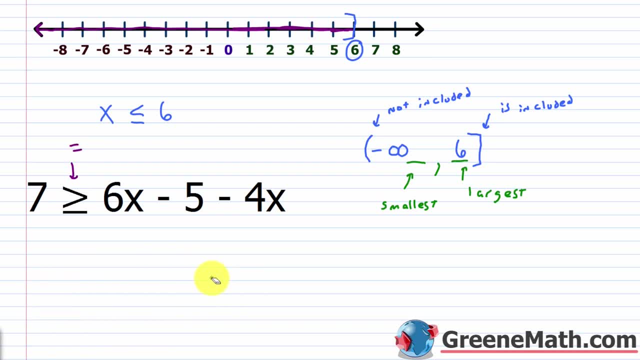 I have some room to work, And so if I did that, I would put: 7 is equal to 6x minus 5 minus 4x. Then just take your solution and do the same thing. Replace the inequality symbol with equals. 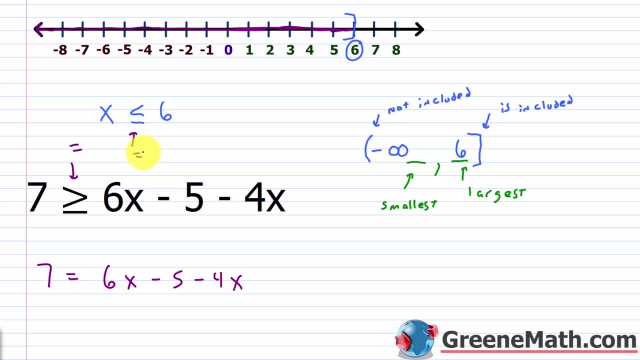 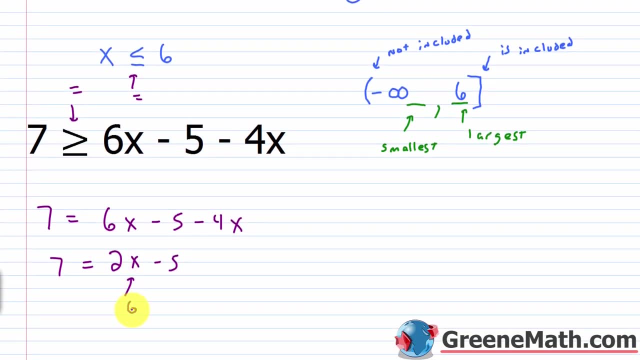 So if I put a 6 in for x, do I get a true statement? So this would be: 2x minus 5 equals 7.. If I plugged in a 6 there, 2 times 6 is 12.. 12 minus 5 is 7.. 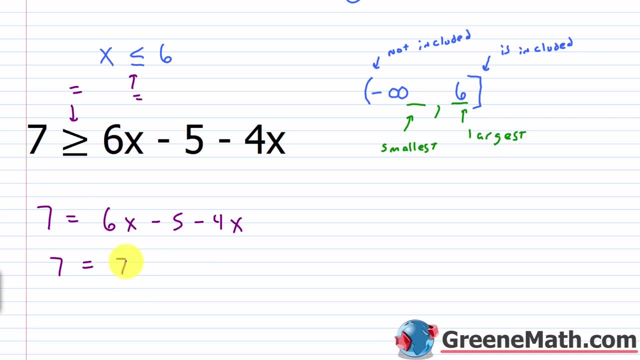 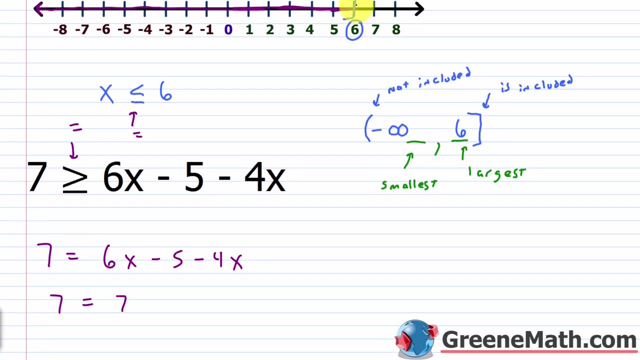 So, yes, that works out. So 6 is your boundary point. It separates the solution region from the non-solution region. You can even see that graphically At 6, we have a separation where 6 works and anything to the left of 6. 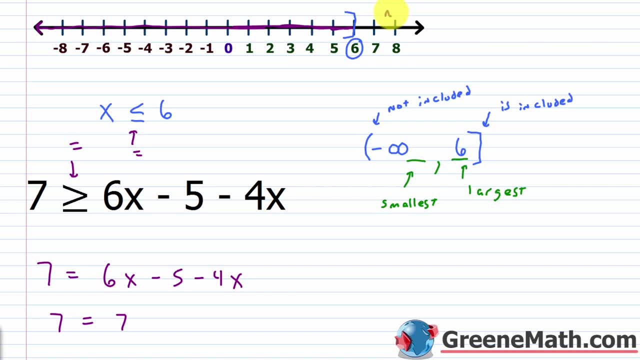 works, but anything to the right of 6 doesn't. So this is a non-solution region, But here is a solution region. So 6 is your boundary, And you'll hear me talk about that. a lot moving forward Now once you've established that. 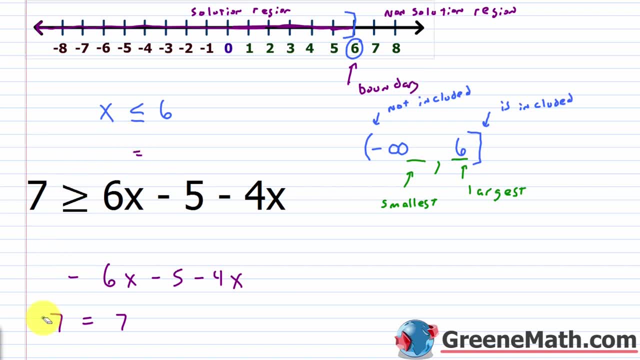 you just check a number on each side. So we'll do that with the inequality there And I'm just going to simplify the inequality and make it a little easier for us. So 7 is greater than or equal to. we know this would be 2x minus 5.. 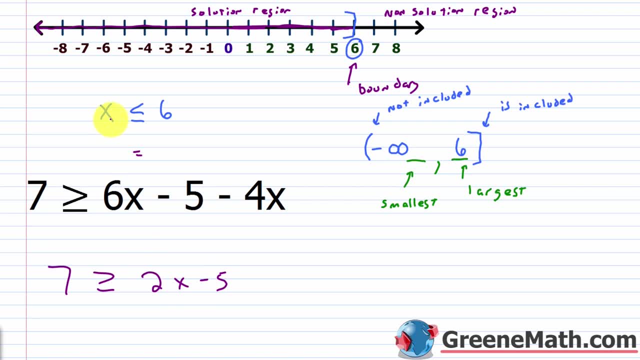 If I check 8, it shouldn't work because x has to be less than or equal to 6.. So if I plugged in an 8 there, I'd get 16 minus 5, which is 11.. So 7 is greater than or equal to 11.. That's false. 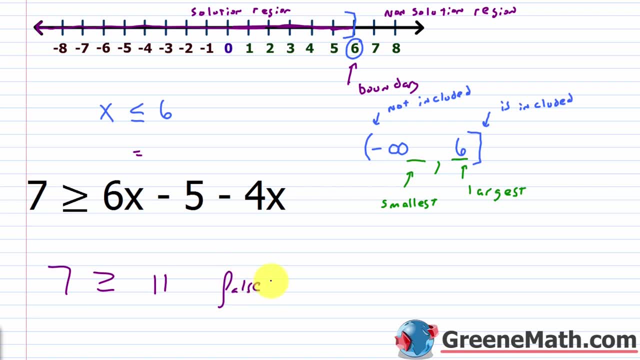 That's what we expect. 8 should not work because we're saying x has to take on a value that's less than or equal to 6.. So that's good. Now the next thing we want to do is we want to check a value. 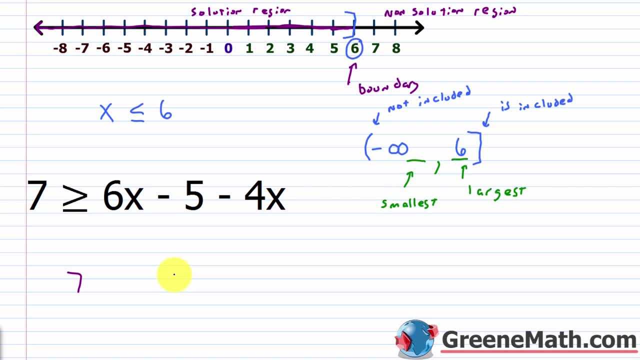 that is less than the number 6.. So let's check 5.. So 7 is greater than or equal to 6.. Again, this simplifies to 2x minus 5.. If I plug in a 5 for x, I get 2 times 5,. 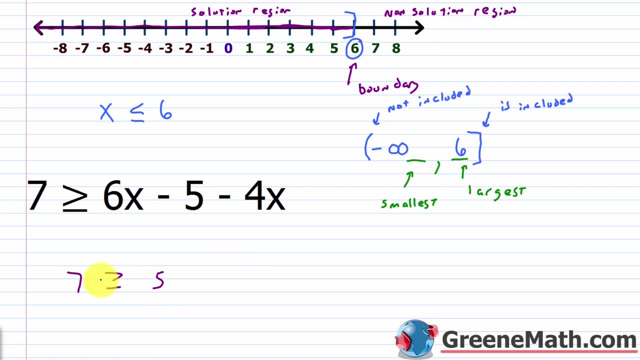 which is 10.. 10 minus 5 is 5.. So I get 7 is greater than or equal to 5, and that is true. 7 is certainly greater than 5.. So you can see that it's more tedious to check these. 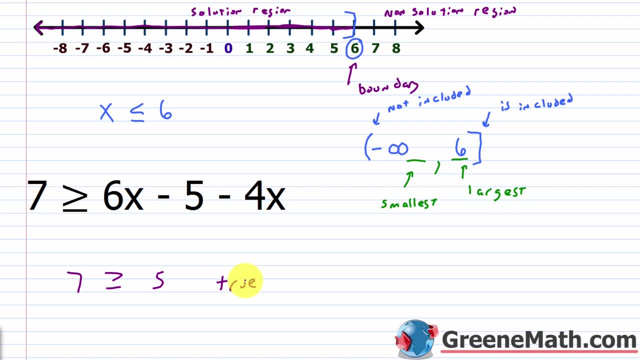 You've got to establish the boundary and then you've got to check 1 on each side of the boundary, So 1 in the non-solution region. We checked 8, and it didn't work. so that's right Then. 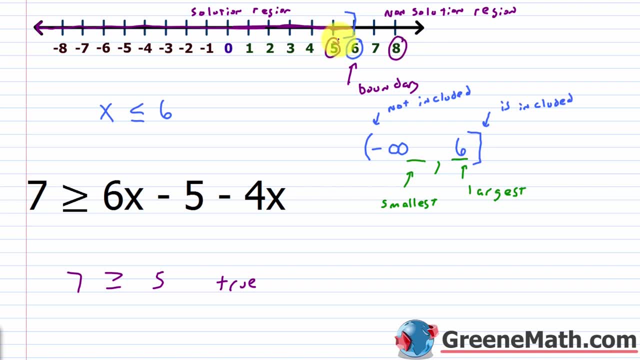 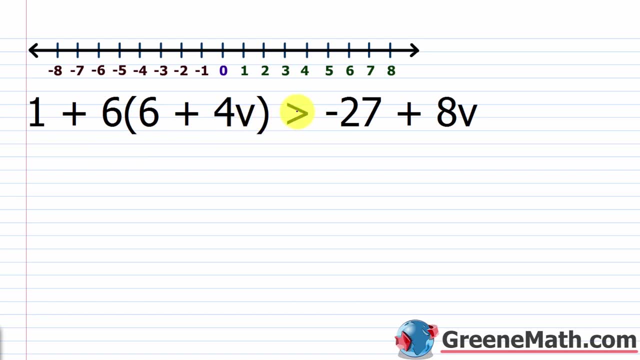 1 in the solution region. We checked 5, that worked, so that was right. Alright, so let's kind of roll through these now. So I have 1 plus 6 times the quantity 6 plus 4v, and this is greater than. 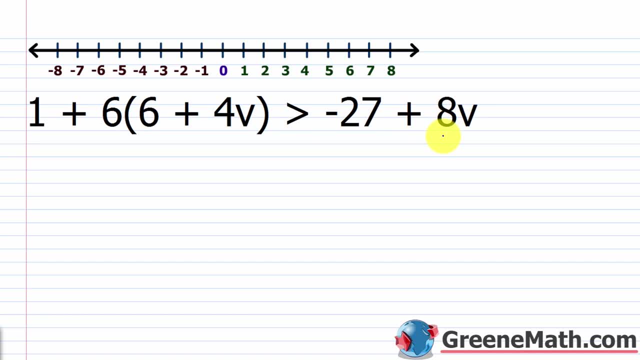 negative: 27 plus 8v. Alright, so let's simplify each side now. So we have: 1 plus 6 times 6 is 36, plus 6 times 4v is 24v, and this is greater than. 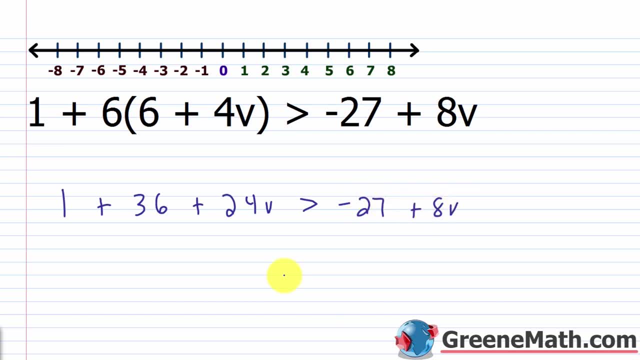 negative 27 plus 8v. So 1 plus 36 is 37, plus 24v is greater than negative 27 plus 8v. So let's subtract 8v from each side of the inequality and let's subtract 37 away from each side. 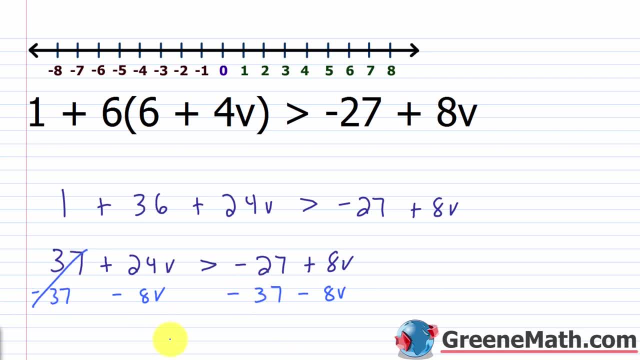 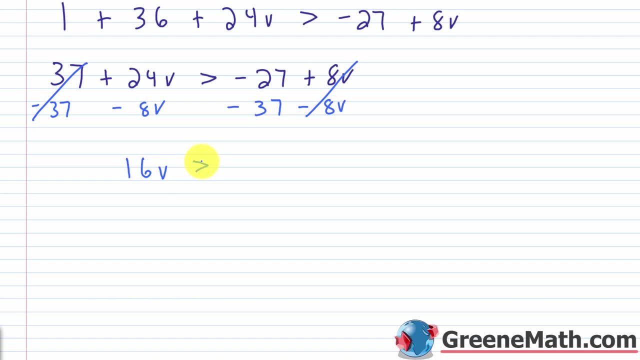 of the inequality. So this is going to cancel and this is going to cancel. 24v minus 8v is 16v and this is greater than negative. 27 minus 37 is negative 64. So to get v by itself, I divide both. 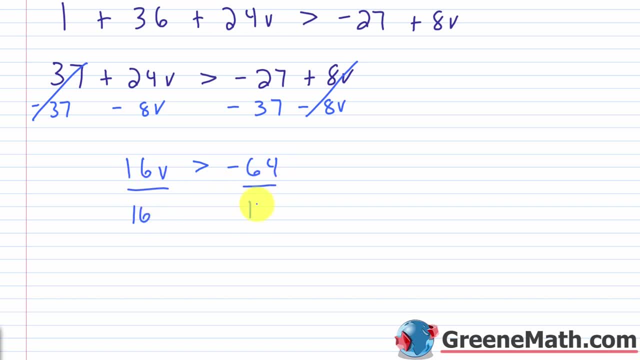 sides by 16, and I'm dividing by a positive there, so I don't have to do anything special. So this cancels with this and I get v is greater than we have negative 64 over 16,, which is negative 4.. 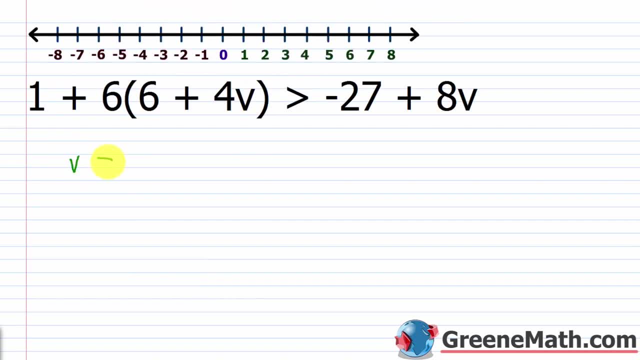 So let me erase everything real quick. So again we found that v was greater than negative 4. So typically your book or your teacher is going to ask you to do two things. once you get a solution Again, write it in interval notation. 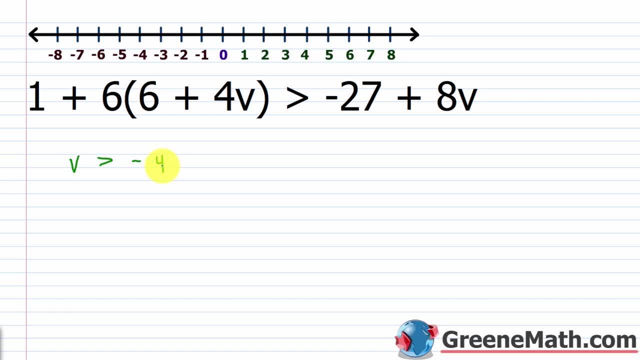 and graph it. So in interval notation again we have these two blanks where we have the smallest and we have the largest And technically I'm going to put what Negative 4 here is the smallest. Is negative 4 actually the smallest value? 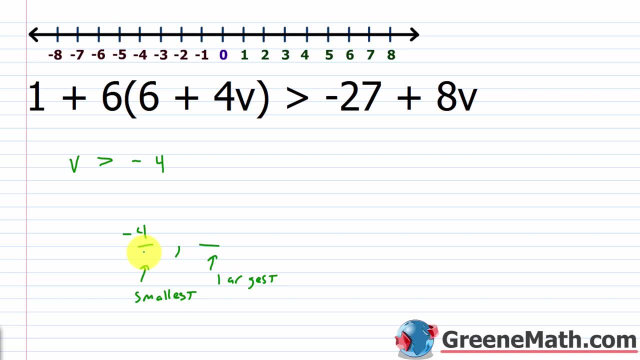 that v can take on. No, it's not. It's as close as we can get to thinking about it, though I can't possibly live with just the smallest value To show that I'm going to put a parenthesis next to negative 4.. 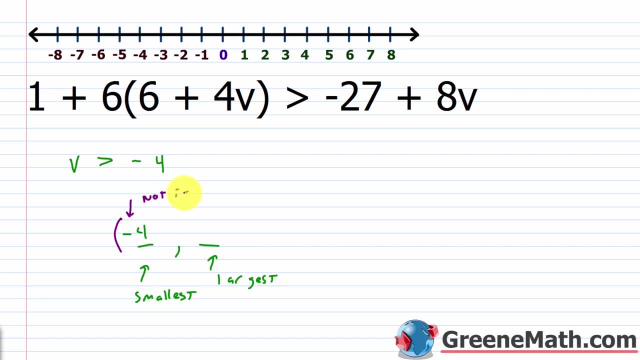 Let's say it's not included. But anything larger than negative 4 would work. If I had negative 3.999999978, that would work Because looking at a number line, that would be larger than negative 4.. But again, 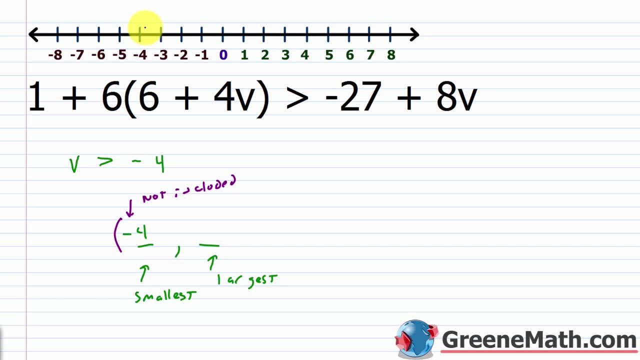 anything that's negative 4 or smaller will not satisfy the inequality. What about the largest value that this can take on? Well, again, because this is going to go forever and ever and ever in the right direction, we use infinity, And with infinity. 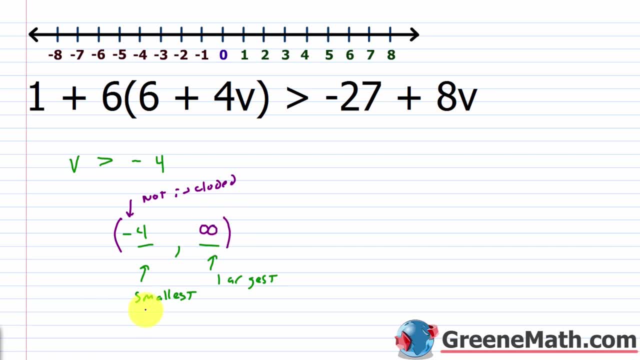 we always use a parenthesis, So again, it's not the smallest number technically, but we use this concept to notate things. So anything larger than negative 4 up to infinity. Now, graphically, we would show this in a similar way. 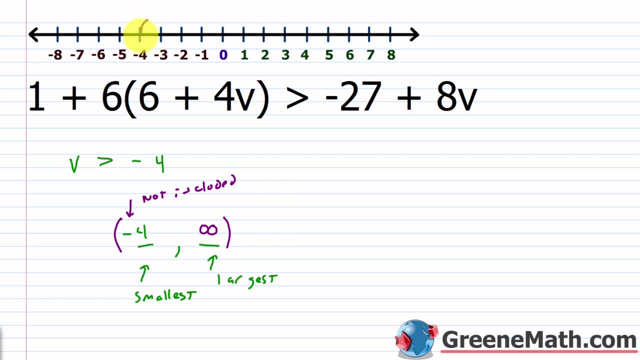 Negative 4 is not included. so I put a parenthesis at faces to the right And then I would shade everything to the right, Everything in the solution region, Including that arrow, to say, hey, this continues forever and ever and ever. Some people will even put an infinity. 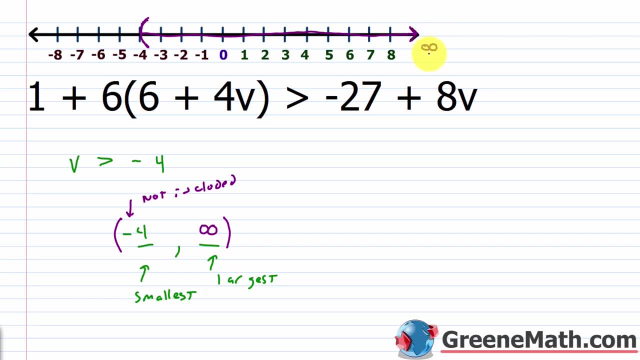 out here to show that And additionally, you might see this in your textbook. You might see an open circle like this. It's open to show that negative 4 is not part of the solution set Alright for the next one. we're looking at 6 times. 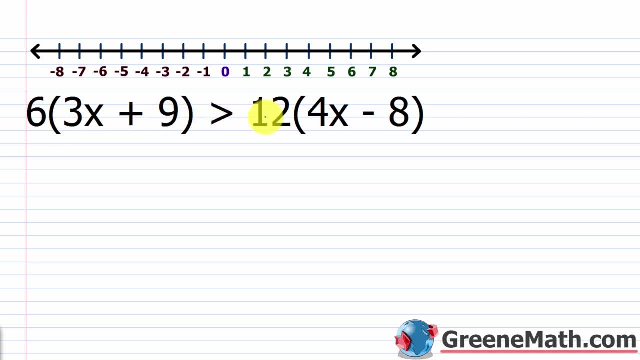 the quantity 3x plus 9 is greater than 12 times the quantity 4x minus 8.. So 6 times 3x is 18x, Plus 6 times 9 is 54. This is greater than 12 times 4x is 48x. 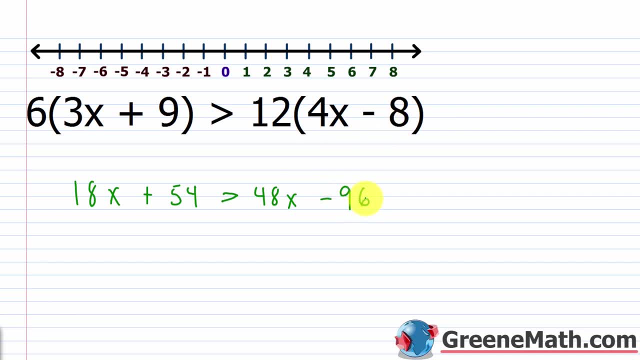 And then minus 12 times 8 is 96. So I want to subtract 48x away from each side of the inequality, And I know that this is going to cancel. I also want to subtract 54 away from each side of the inequality. 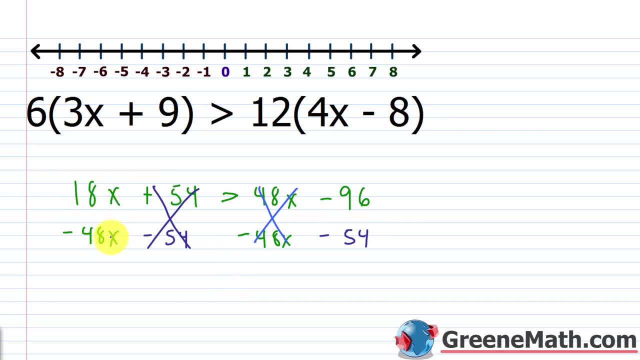 This is going to cancel. 18x minus 48x would be negative 30x, And this is greater than negative. 96 minus 54 is negative 150.. So now to get x by itself. I'm going to divide both sides. 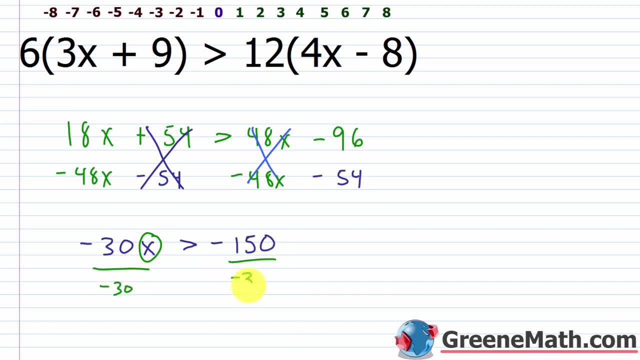 by negative 30. But remember I'm dividing both sides by a negative, so this has to be flipped. Right now it is a greater than I flip the direction, it's going to become a less than. So x is going to be less than. 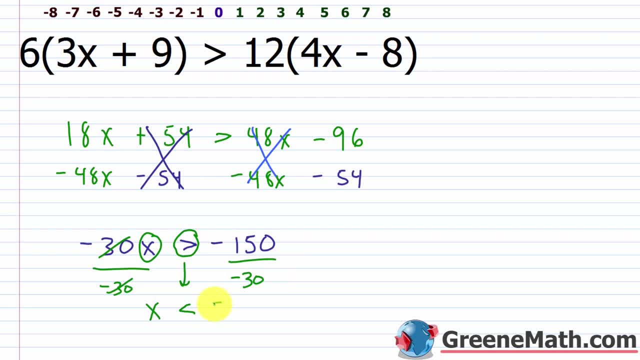 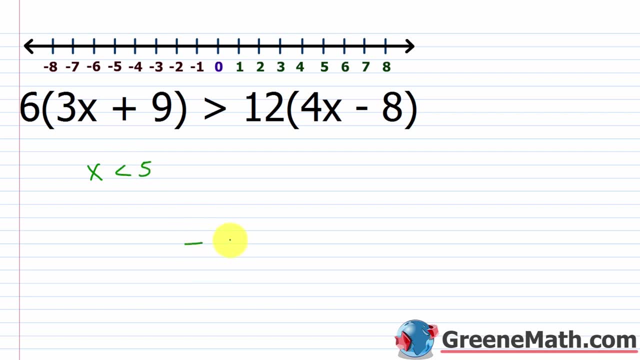 negative 150 over negative 30 is going to be 5.. Let's erase everything. So again we have that x is less than 5.. In interval notation, again we think about this concept of a smallest value and a largest value, And again that's. 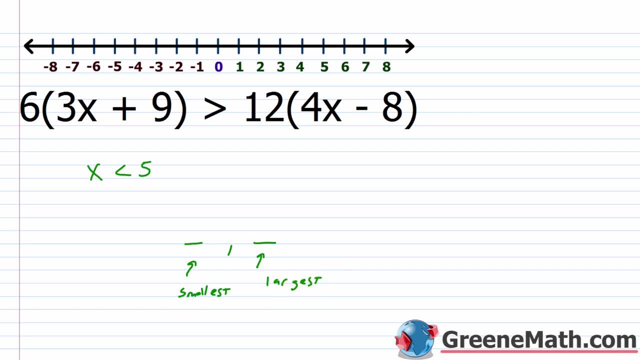 not technically correct. That's how we think about it. So x is less than 5.. The largest value that this can take on is not 5. But anything smaller than that, So 4.99999999978, for example. So I put a parenthesis. 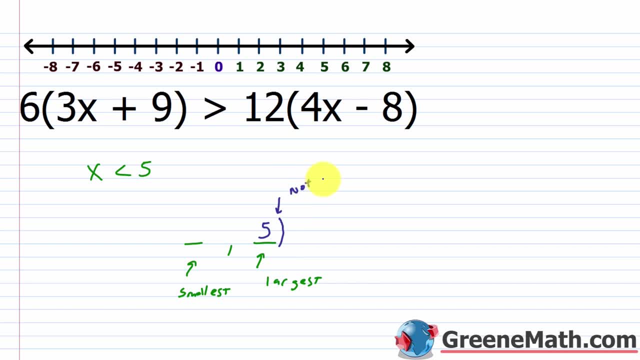 next to 5, just to say that it's not included. What's the smallest value this can take on? Well, it's going to continue forever and ever and ever in the left direction, because it's anything less than 5.. So negative 1 trillion, for example. 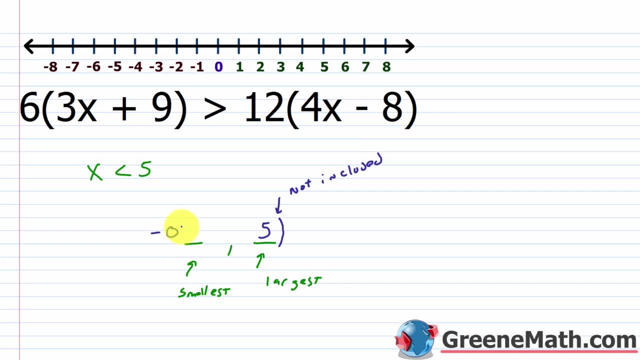 would be a solution. So I use negative infinity. And again, if I use positive or negative infinity, I always put a parenthesis next to it. Now, graphically, x is less than 5. Find 5 and put a parenthesis that faces left. 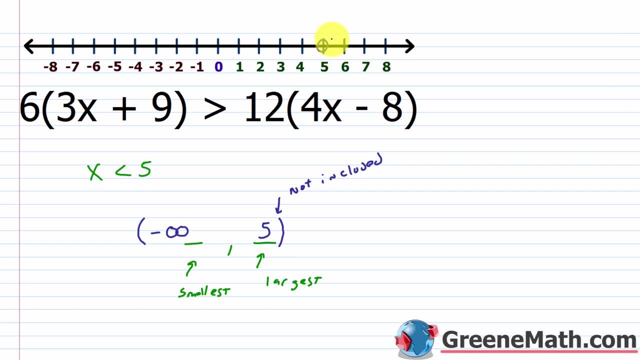 or put your open circle again to show that 5 is not included. Either one- And then shade everything to the left. So you shade all this in the solution region, including the arrow, And again some people like to put a negative infinity out. 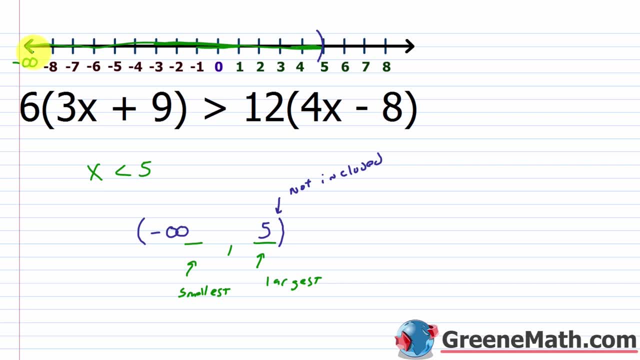 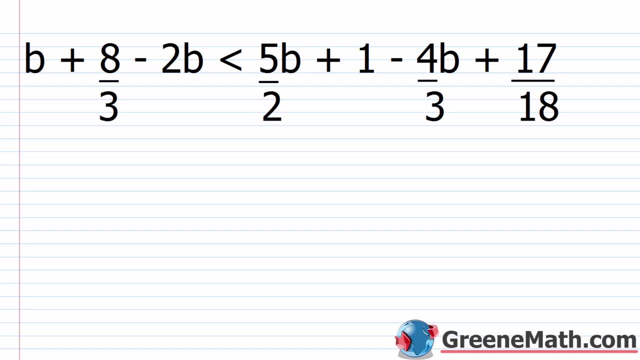 here to show that it's just going forever and ever and ever in that direction. Alright, so we also have ones that have fractions involved. So, just like we saw with equations, we can multiply both sides by the LCD. Now I'm going to simplify. 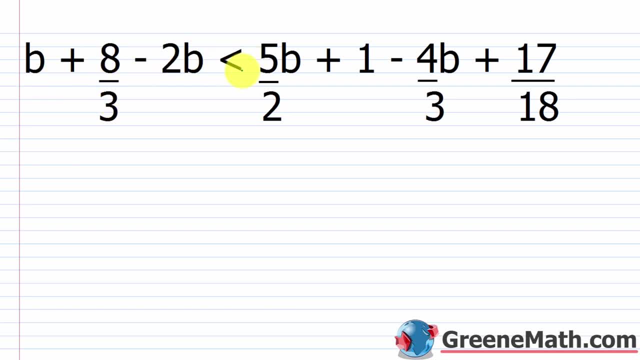 before I start. So we have b plus 8. thirds minus 2b is less than 5 halves. b plus 1 minus 4 thirds. b plus 17 eighteenths. What can I do? Well, I know, b minus 2b. 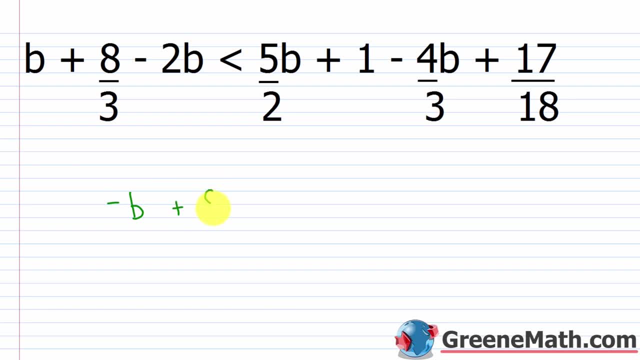 would be negative b Negative b plus 8 thirds is less than nothing really I can do here without working with fractions. so let's just write 5 halves b plus 1 minus 4 thirds b plus 17 eighteenths. What would my LCD be? 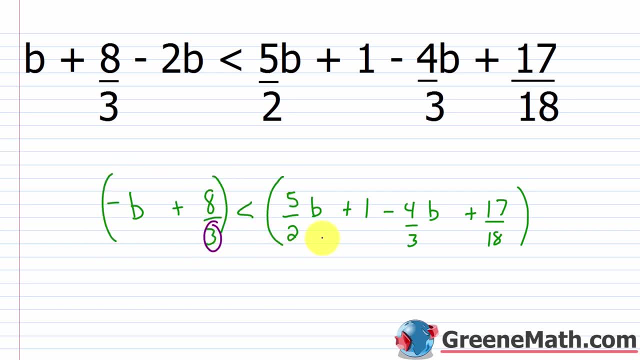 here I'm looking at denominators of 3,, 2,, 3, and 18.. Obviously, it's going to be 18.. So we're going to multiply both sides of the inequality by positive 18, so I don't need to flip anything. 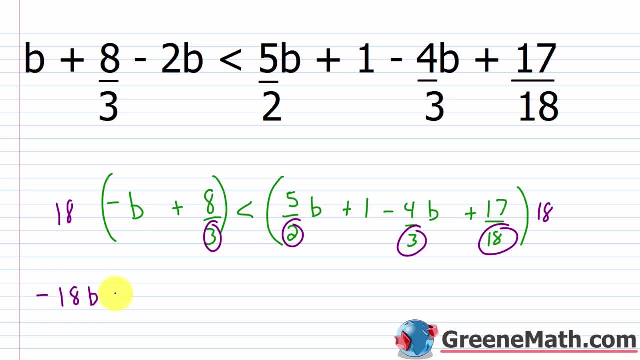 18 times negative. b is negative 18b plus 18 times 8. thirds 18 would cancel with 3 and give me 6.. 6 times 8 is 48. This is less than if I have 18 times 5 halves. 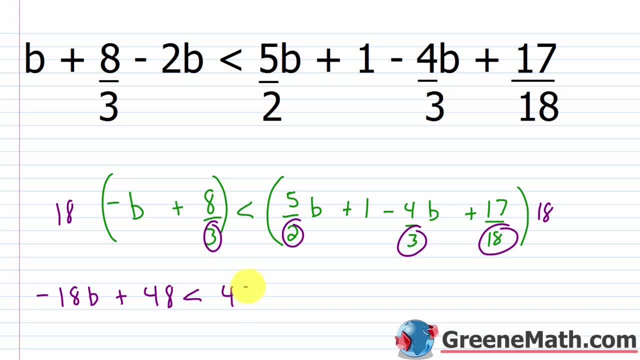 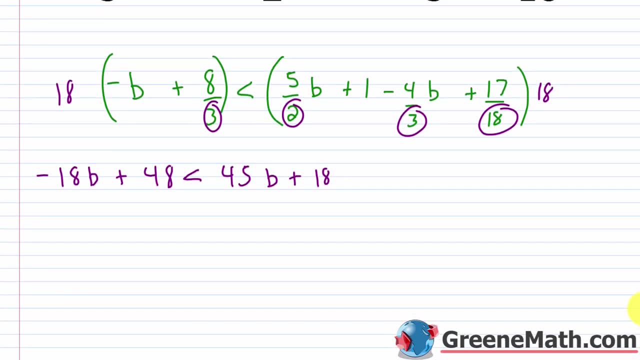 18 would cancel with 2 and give me 9.. 9 times 5 is 45, then times b plus 18 times 1 is 18. then we have 18 times negative 4 thirds b. We know that's negative 18 divided by 3. 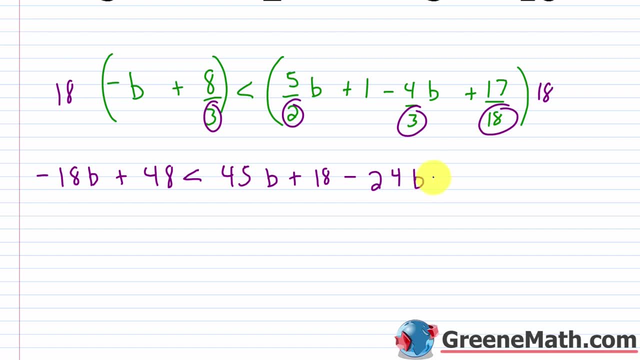 is 6.. 6 times 4 is 24, so minus 24b. Then, lastly, plus 18 times 17. eighteenths, 18s would cancel. you just have 17.. Alright, So nice and easy now. 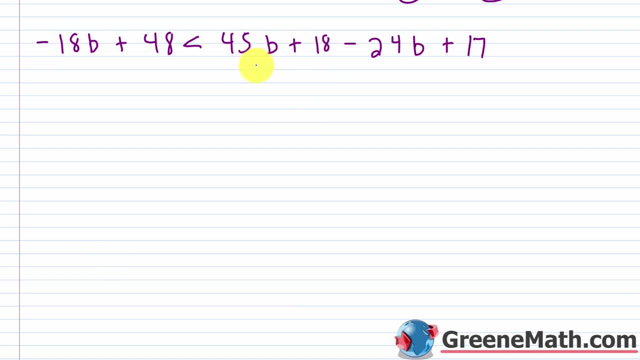 On this side I can do a lot of combining: 45 minus 24 is 21. So 45b minus 24b is 21b, Then 18 plus 17 is 35. And over here I still have my negative. 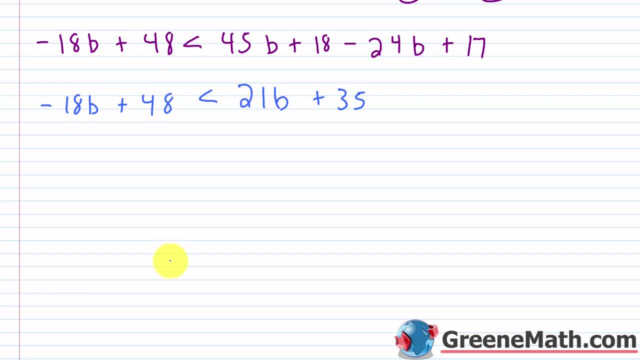 18b plus 48. So I want all of my variable terms on one side, all the numbers on the other. So let me go ahead and subtract 48 away from each side of the inequality. That's going to cancel. And let me also 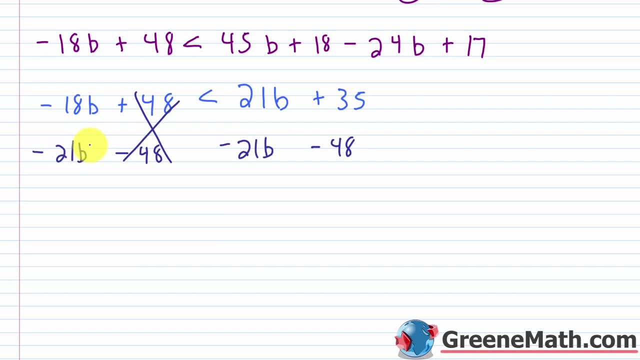 subtract 21b away from each side of the inequality, So that's going to cancel. If I do negative 18b minus 21b, that's going to give me negative 39b And this is less than 35 minus 48 is negative 13.. 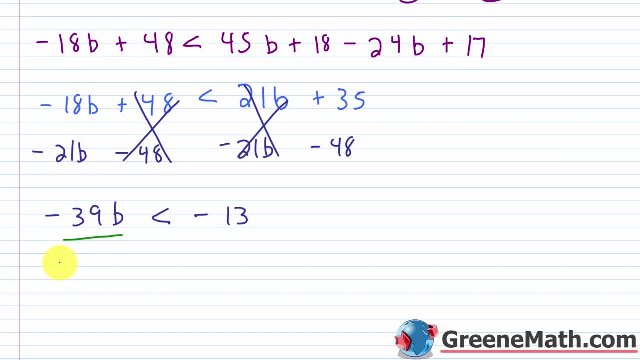 So now we divide both sides of the inequality by negative 39. And again, if I'm dividing by a negative or I'm multiplying by a negative, this has to be flipped. So this becomes greater than from a less than So this cancels and I've got. b is greater than. 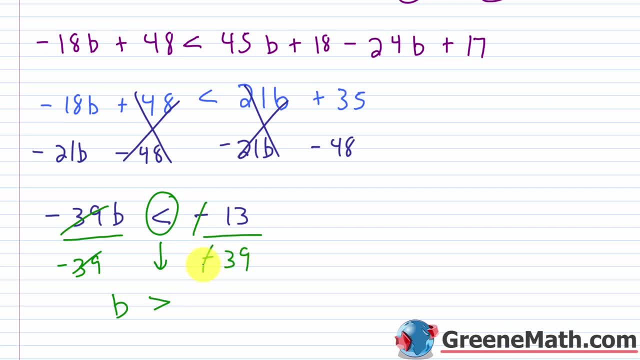 negative 13 over negative 39. the negatives cancel 13 over 39. each is divisible by 13, so you get one third. So b is greater than one third. So again we have that b is greater than one third. So we can start out with. 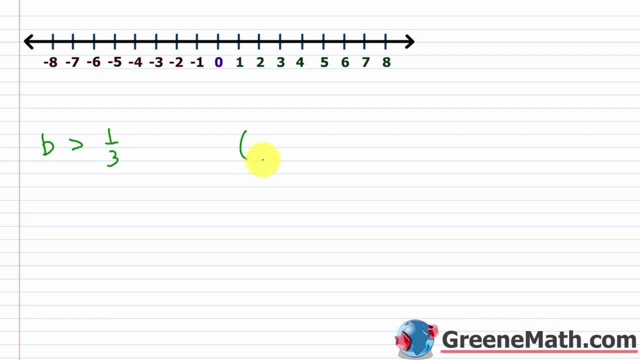 interval notation. Again, on the left, we want the smallest value. Now, one third is not technically the smallest value, but we're putting it in there next to a parenthesis to say that it's not included- But anything larger than one third, even if it's a small amount, larger than one third. 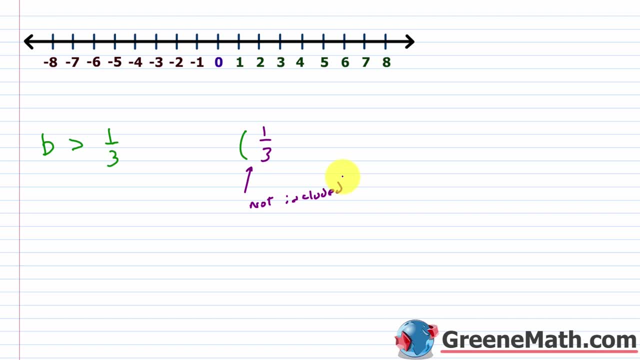 a microscopic amount larger than one third would work. So one third is not included, then comma. This continues forever and ever and ever in the right direction. So we put infinity here, We put a parenthesis there. We always use a parenthesis with infinity. 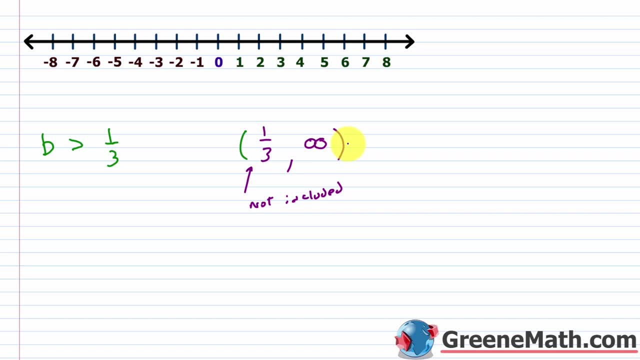 So graphically, I would find one third. Now I don't have a notch for that, so I'm going to create one. Let's just say one third is about right there. Let's say: this is one third, And I'm going to put a parenthesis. 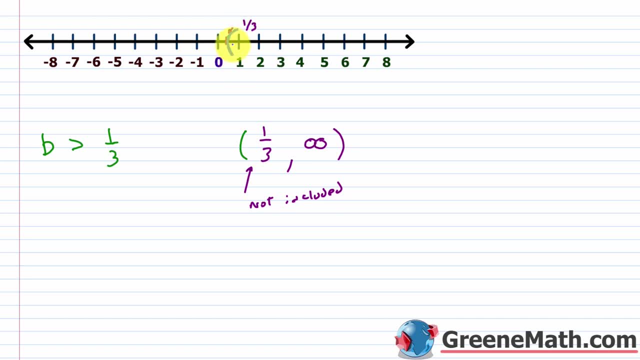 there, Or again you can use that open circle technique, Doesn't matter. And then I'm going to shade everything to the right, Everything in the solution region, including that arrow, And again you can put an infinity out here to say one third is not. 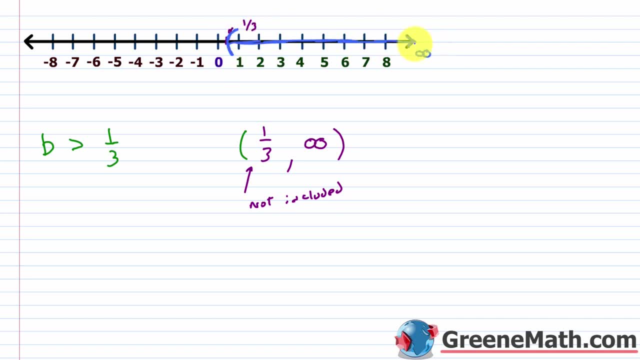 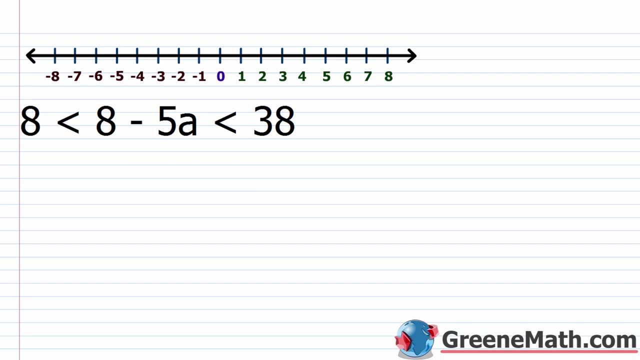 included, But anything larger than one third works as a solution for this inequality, Alright. so the last thing we want to cover is a three part inequality. So we saw these in Algebra 1.. And basically what happens is you have this guy in between. 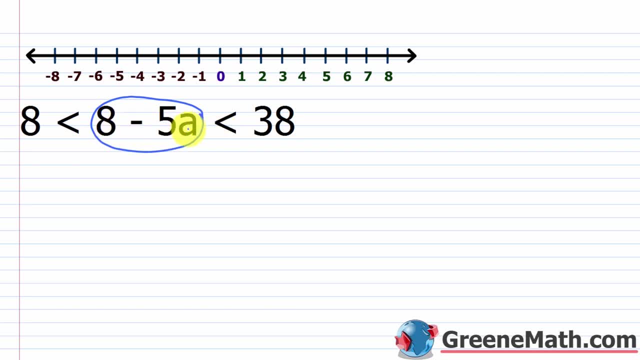 two inequality symbols. So 8 minus 5a is greater than 8. And it's less than 38. So both the conditions have to be met. So what's going to happen is you're going to do one of two things. You can separate these. 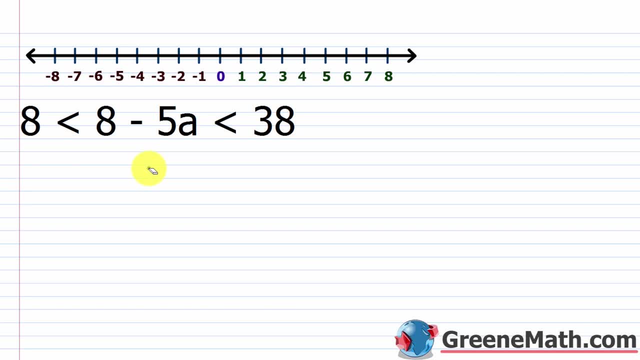 and solve them And then put it back together in the end, which is more work, Or you can solve it doing the same thing to each part. So, in other words, I want to isolate a in the middle. So what I do is I subtract 8. 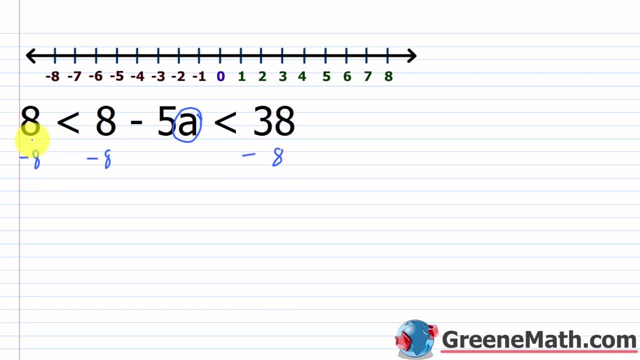 away from each side to begin. So then 8 minus 8 is 0. And this is less than This would be 0. So I'd have negative 5a, And then less than 38 minus 8 is 30.. 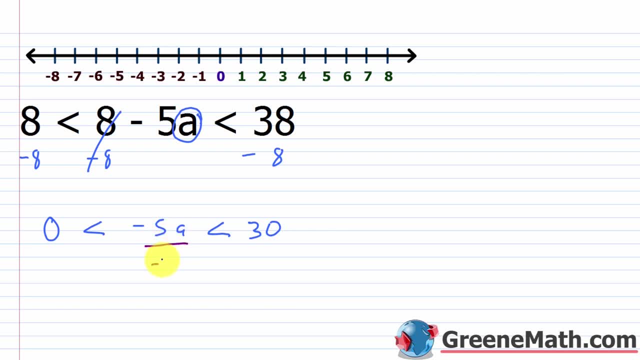 Now, if I want a by itself, I would divide each part by negative 5.. But remember, if I'm dividing by a negative, I've got to flip the direction of the inequality. Right now these are less than So if I flip the direction of that, 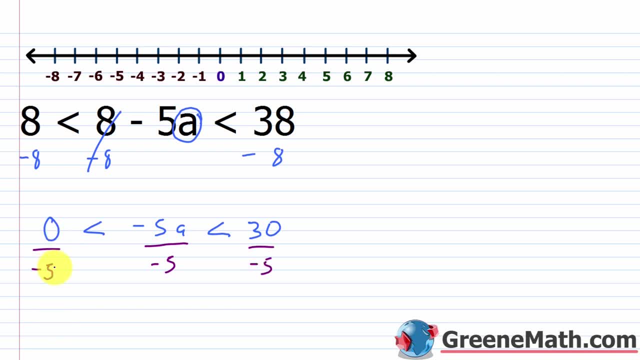 symbol. it's going to become a greater than So. this would be 0 over negative. 5 is 0. I'd have a greater than This would cancel and I'd have a, And then a greater than So. this would be 0 over negative 5 is negative 6.. 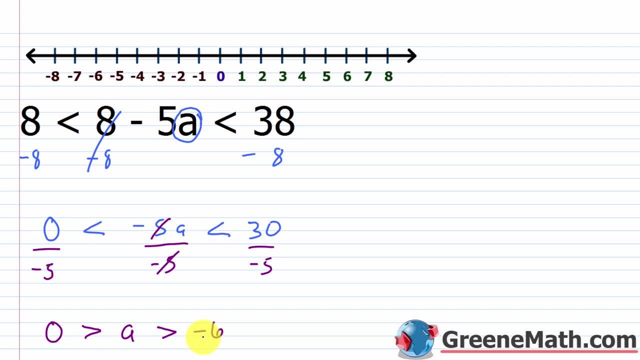 Now you don't want to keep it like this. You want to put it in the direction of the number line. Negative 6 is to the left of 0. So you want it lined up that way. So we would put negative 6. 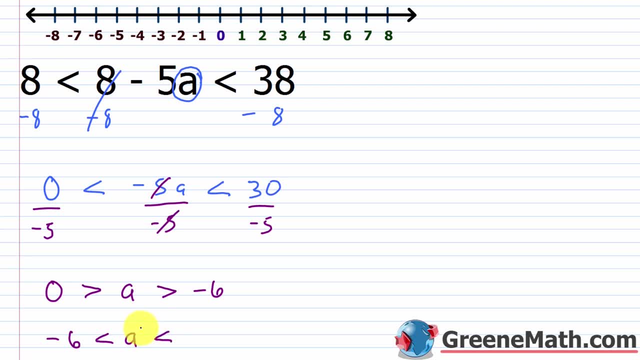 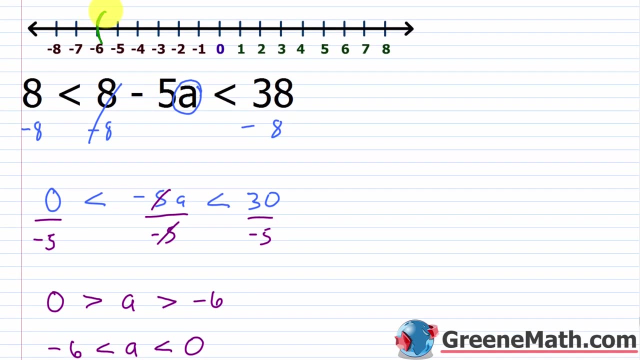 is less than a, which is less than 0. Or a is greater than negative 6, and also it's less than 0. Looking at a number line, it's a range of values not including negative 6. So I'd put a parenthesis there. 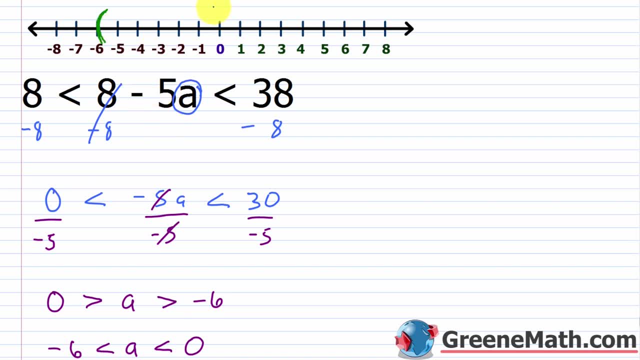 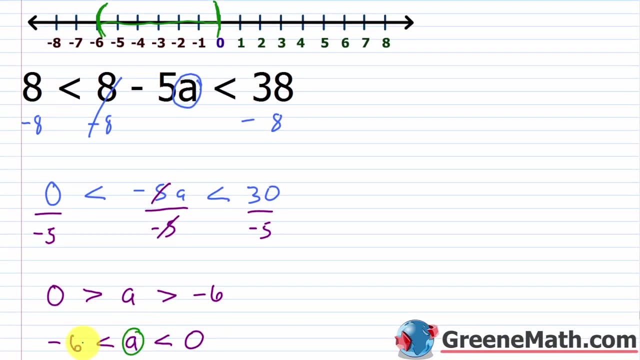 So anything larger up to, but not including 0.. So I'd put a parenthesis there. I would shade everything in between. This is just telling me that a is a value that's between negative 6 and 0.. In interval notation, again, we use this: 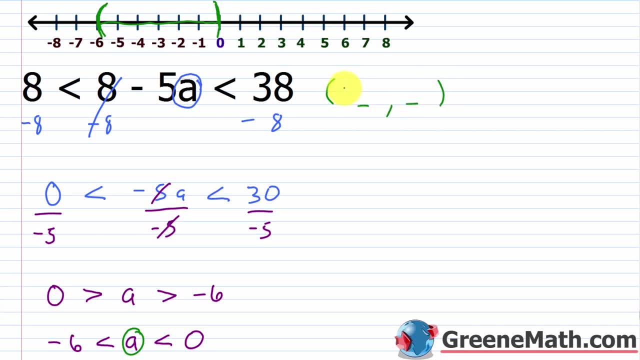 concept of the smallest and the largest negative. 6 would go in this spot for the smallest. It's not included, so I put a parenthesis there. 0 would go in the spot for the largest. It's also not included, so I put a parenthesis there. 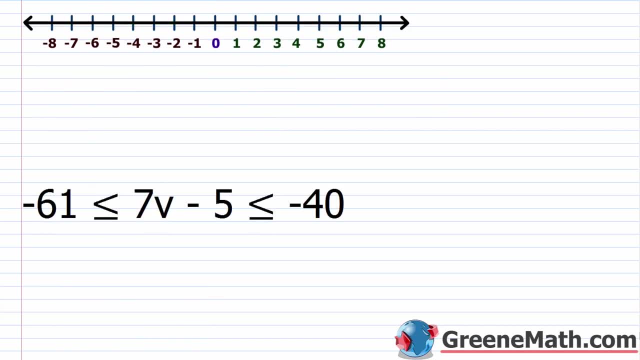 So here's interval notation and here's graphically Alright. let's look at one final problem, And again, these three part inequalities are no more difficult. So we have: 7v-5 is greater than or equal to negative 61, and it's less than or equal to negative 40.. 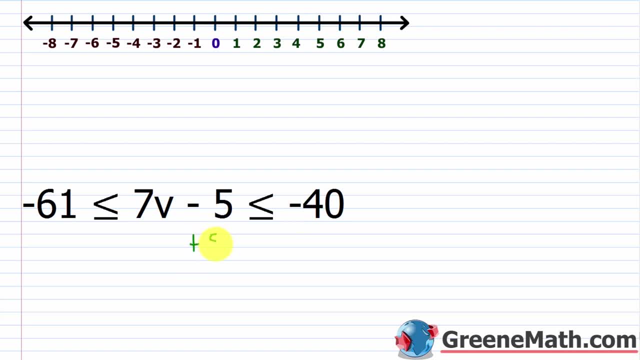 So again, do the same thing to each side. So plus 5 here, plus 5 here, plus 5 here. So negative 61 plus 5 is going to give me negative 56. And it's less than or equal to this cancels. so I'll just have 7v. 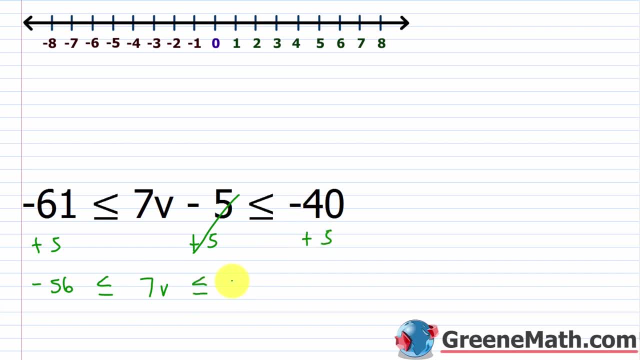 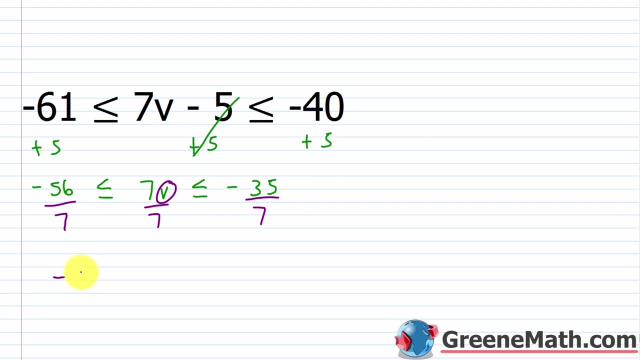 and it's less than or equal to negative. 40 plus 5 is negative 35.. So now what I want to do is divide each part by 7 so I can isolate v, and what's going to happen is negative. 56 over 7 is negative 8. 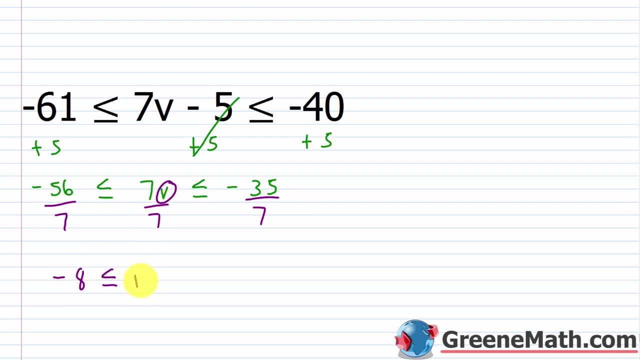 this is less than or equal to- we'll have v by itself now, because this cancels. and this is less than or equal to: 35 over 7 is negative 5.. So v is greater than or equal to negative 8 and it's less than or equal to negative 5.. 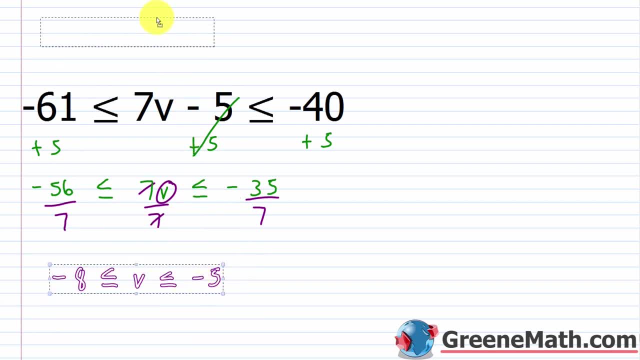 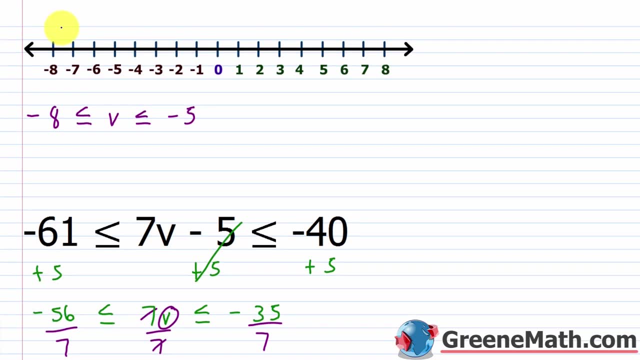 Let me drag this solution up So graphically. if I located negative 8, it's there, So it's included in the solution set. so I'm going to put a bracket here that faces to the right. Same thing with negative 5: it's included. 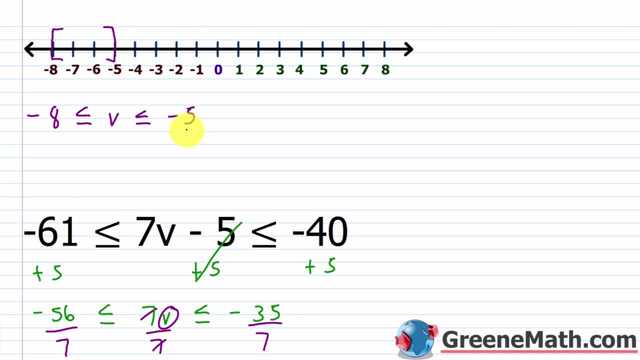 in the solution set, so I'm going to put a bracket there. This one's going to face to the left and I shade everything in between. So what this is telling me is that v can be any value, starting from negative 8, going up to and including negative 5.. 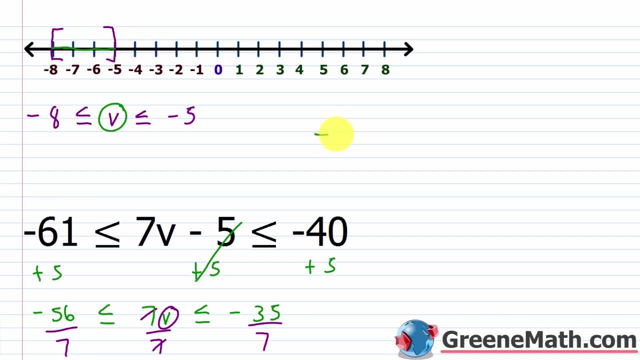 Now in interval notation, again, smallest, largest, let's think about that. the smallest value v can take on is negative 8.. Now negative 8 is included. it's part of the solution. so I use a bracket And it goes up to and includes negative 5.. 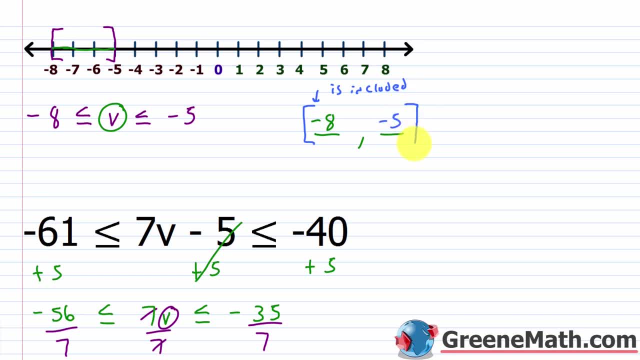 So the largest value would be negative 5.. Again, I'm using a bracket because it's included, So your solution here is that v is any value that is greater than or equal to negative 8 and less than or equal to negative 5.. So again starting. 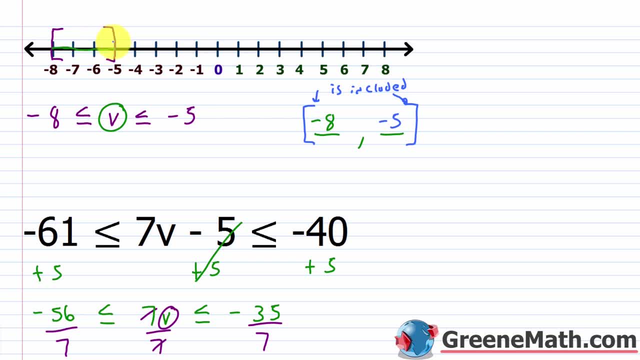 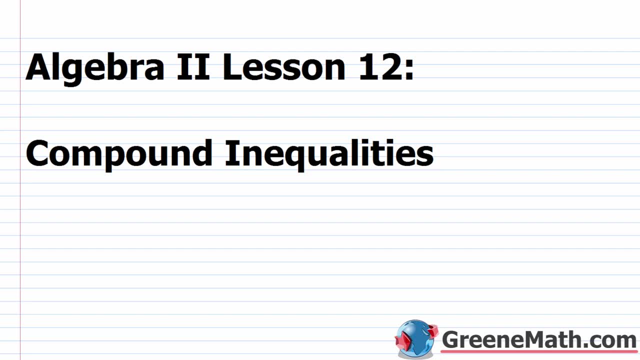 from negative 8, including negative 8, going up to and including negative 5.. Hello and welcome to algebra 2, lesson 12.. In this video we're going to learn about compound inequalities. So in our last lesson we had a review of how to solve a linear inequality. 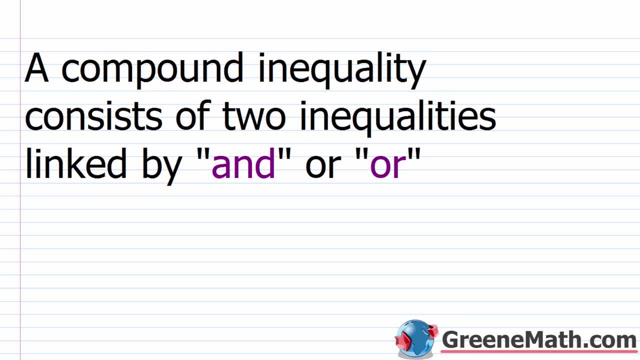 in one variable. Now we're going to move on and look at something that's a little bit more challenging and probably new for you in your algebra 2 course. We're going to talk about compound inequalities. So a compound inequality consists of two inequalities linked. 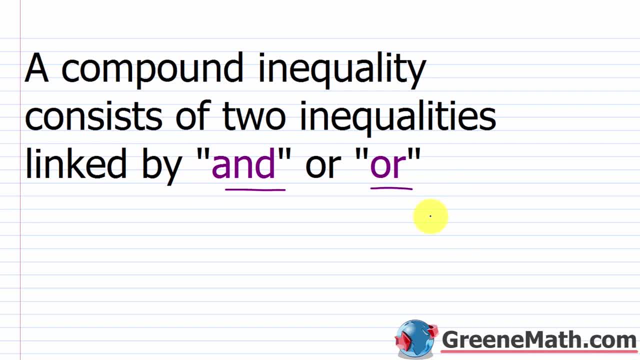 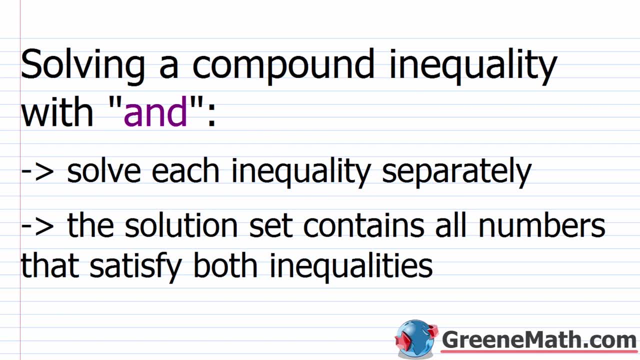 by the word and or the word or. Okay, so those are the two different scenarios. Now, the first one we're going to deal with is solving a compound inequality with, and Now I suggest you get a flashcard, or, if you don't have a flashcard, a piece of loose leaf. 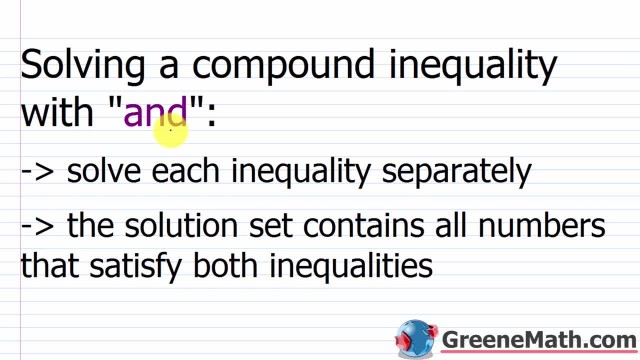 write down the procedure for each one, because they're a little bit different, and then, as you're working through your problems, you can reference your flashcard or your piece of loose leaf- whatever you wrote it down on. after about 20 or so of these, you're going to have this procedure down packed. 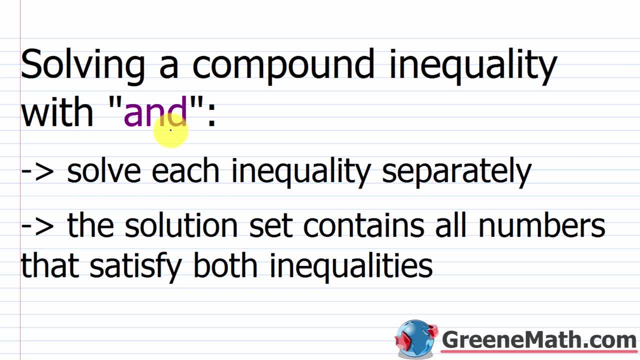 and you won't get confused. So the first thing you want to do with this scenario of and you want to solve each inequality separately. Okay, so just treat it as if it's two separate problems. The next thing you want to do is find the solution set. 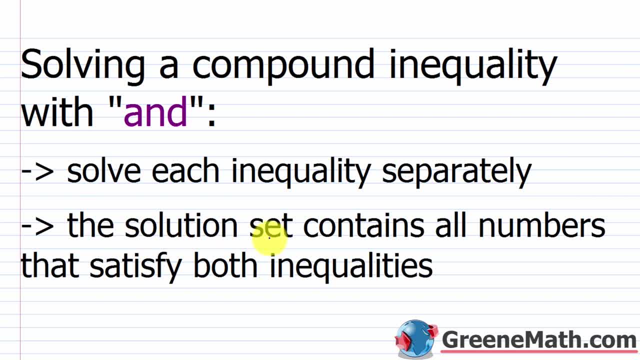 for the compound inequality. Now, the solution set contains all numbers that satisfy both inequalities, Both inequalities. So if it's not a solution to both, it's not a solution for the compound inequality. And a good example of this: remember when we started talking about sets at the very beginning. 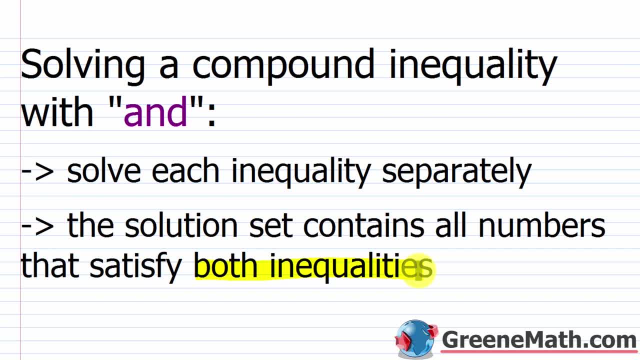 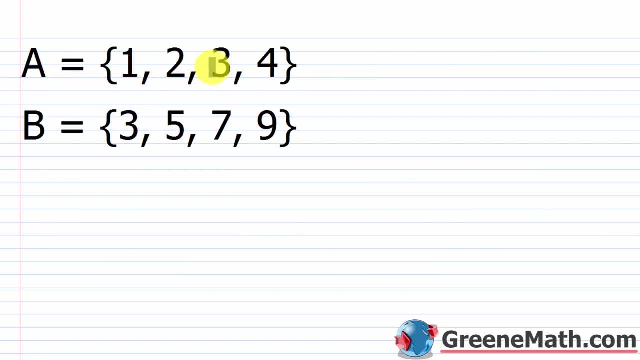 of Algebra 2, we talked about the intersection of two sets. So as an example of that, I have two basic sets here. I have set A, which contains the elements 1,, 2,, 3, and 4.. And I have set B, which contains the elements: 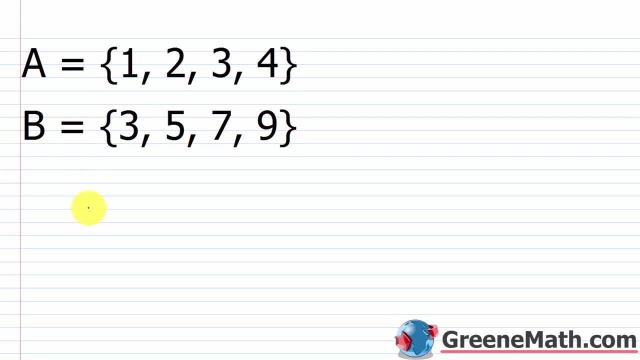 3,, 5,, 7, and 9.. So if I'm looking for the elements that are common to both, I'm looking for something known as the intersection of the two sets, So A and B, I want the intersection of the two. This is the symbol for that. 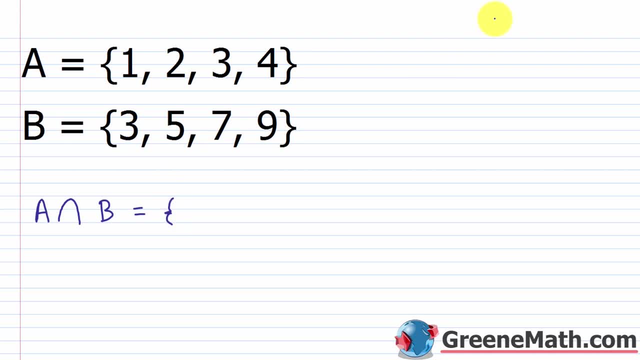 And this contains all the elements that are common to both. Well, if you look through here, it's just three. This is the only element that's common to both. So this set contains one element, and that element is 3.. And when we're solving this compound inequality with AND. 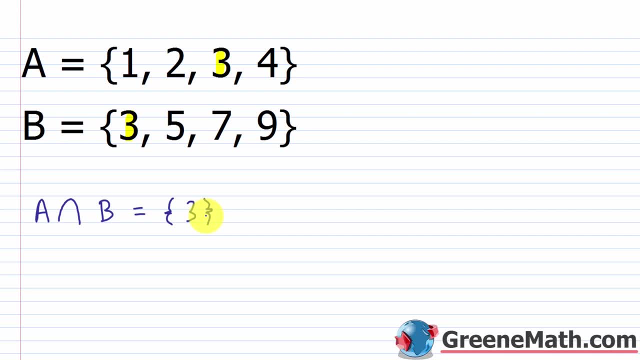 we're doing the same thing. We're looking for the intersection of the two solution sets. Alright, so let's get started with the first problem, And we already know how to solve a linear inequality in one variable. That part is simple: It's just putting the two together. 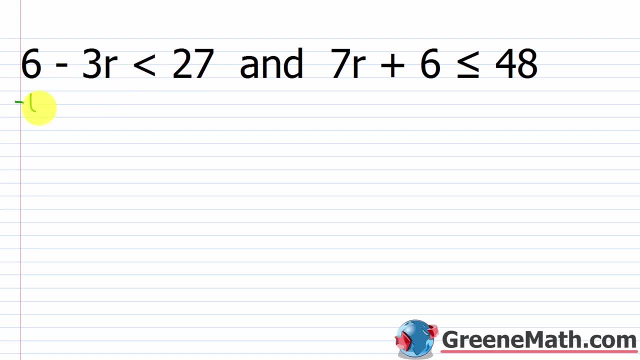 Alright. so if I have 6 minus 3r is less than 27, I can subtract 6 away from each side of the inequality, So that's going to cancel. I'll have negative. 3r is less than 27 minus 6 is 21.. 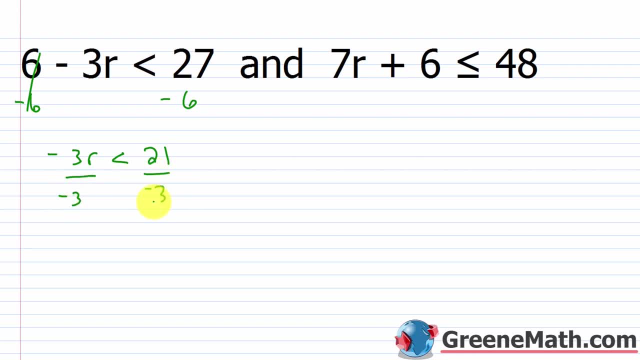 Divide both sides of the inequality by negative 3. Remember, if I divide by a negative, I've got to flip the direction of the inequality symbol. So this is a less than. It's going to become a greater than. So this would cancel with this and I'd have r. 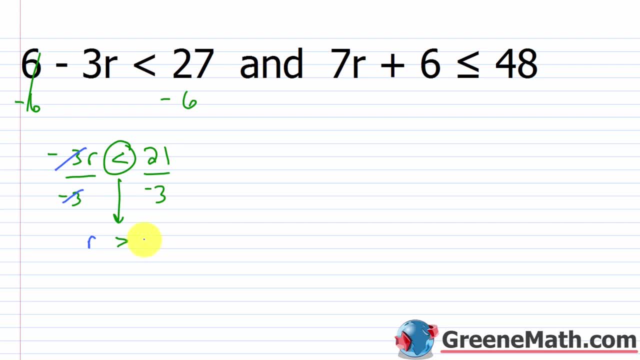 And now it's a greater than 21 divided by negative 3 is negative 7.. Now, over here I'm going to solve this one separately. Let me just put a little line here. I'm going to subtract 6 away from each side. 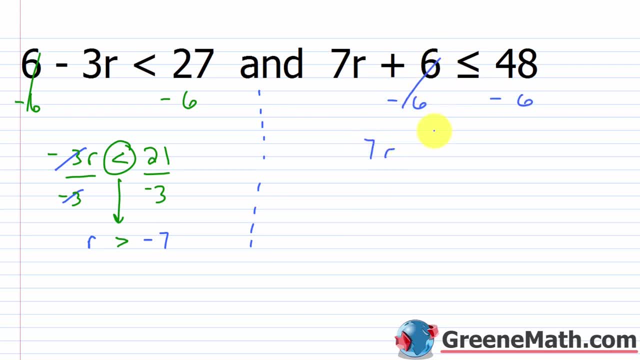 of the inequality. So I'll have: 7r is less than or equal to 48 minus 6 is 42.. I'm going to divide each side by 7. And I'll get that r is less than or equal to 6.. 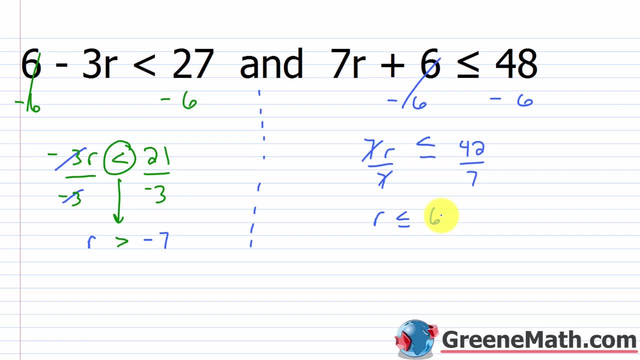 So I have these two solutions. I'm going to go down to where there's a number line. We're going to do the whole song and dance with the interval notation and graphing, And then we're going to put the two solutions sets together. 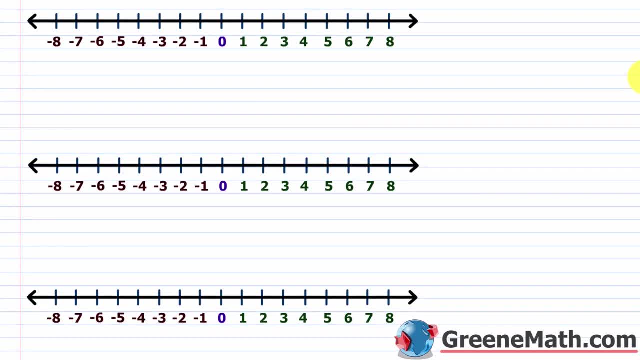 Alright, for the first one. let me just write it out here. We had: 6 minus 3r is less than 27.. We found that for this one r was greater than negative 7. So in interval notation, what does that look like? 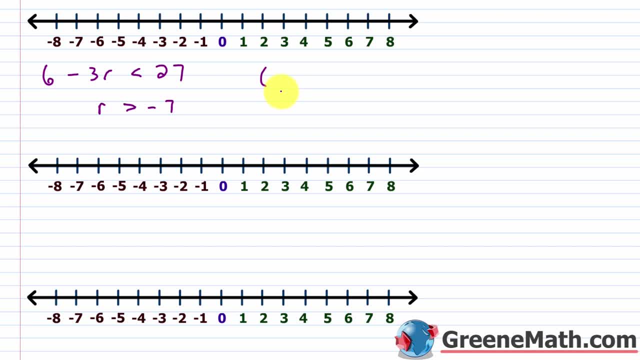 Well, it looks like this: You'd have a parenthesis to say that negative 7 is not included, A comma, and then you'd have an infinity symbol with a parenthesis next to that. So that's interval notation. Graphically on the number line: 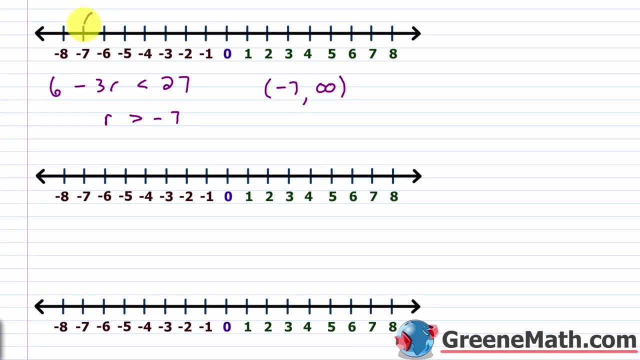 at negative 7. it's not included. I'd put a parenthesis to show that And then I would shade everything going to the right, including that arrow. Now for the next part of the compound inequality. we saw the problem: 7 times r plus 6. 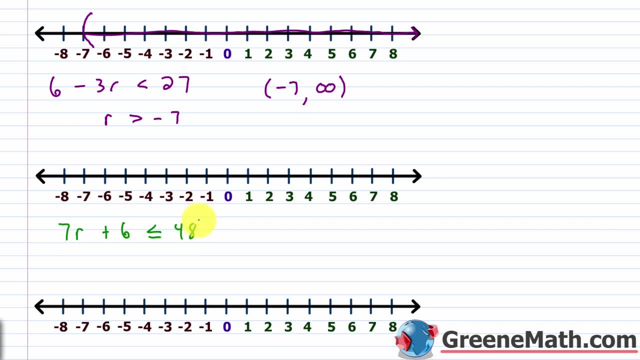 is less than or equal to 48. And what we found there was that r was less than or equal to 6.. So in interval notation, since it's less than or equal to 6, we would have a parenthesis next to negative infinity comma and then up to and including 6.. 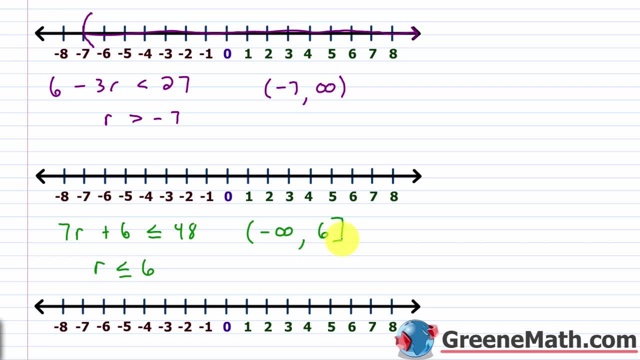 So 6 is going to have a bracket next to it. Alright, now, graphically, at 6 we put a bracket facing to the left and we shade everything going in this direction again, including that arrow. Now for the compound inequality. let me just write this: here we have: 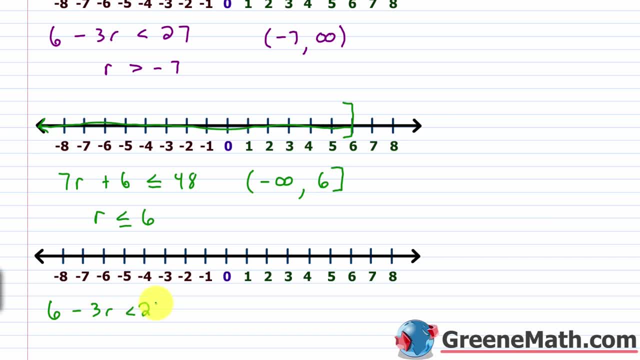 6 minus 3r is less than 27, and then- and we have 7r plus 6 is less than, or equal to 48. So what's the solution here? Well, again, it's the intersection of the two solution sets And for some people, they like to look at it. 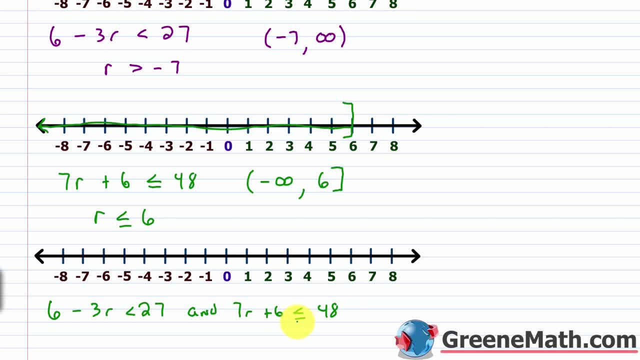 graphically For some people. they like to look at it between the two intervals that were created And some people can just look at it and say, okay, I know it's this. Well, I can tell you that if you just look at the two solutions, 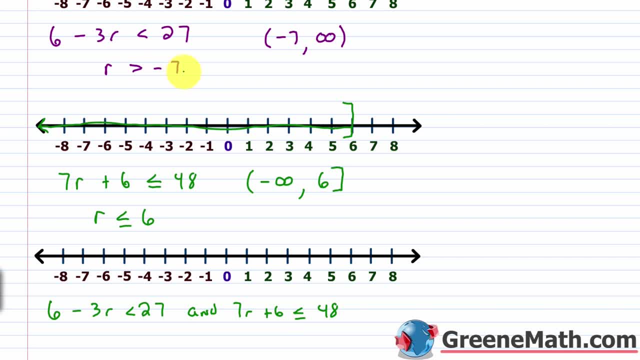 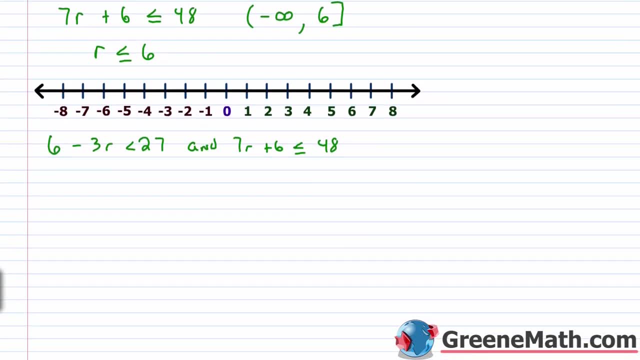 and you put them together: r is greater than negative 7 and r is less than or equal to 6.. So that's pretty easy to do. You can write that as a three part inequality, where you say r is greater than negative 7 and r is also less than. 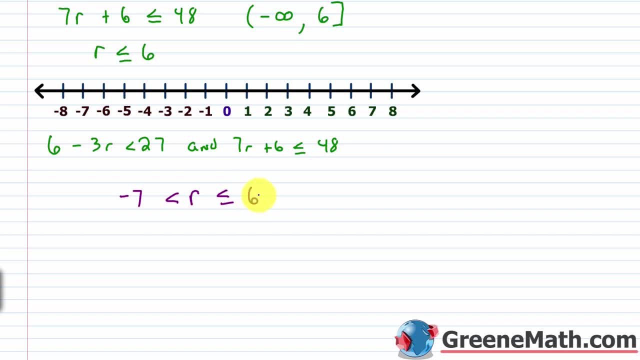 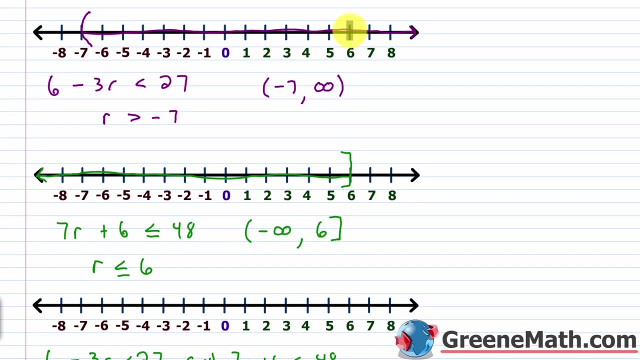 or equal to 6.. In interval notation I would write this with a negative 7 next to a parenthesis to say negative 7 is not included, and then comma, you have a 6 which is included. so that gets a bracket. Now graphically it's easy to tell what it would have been. 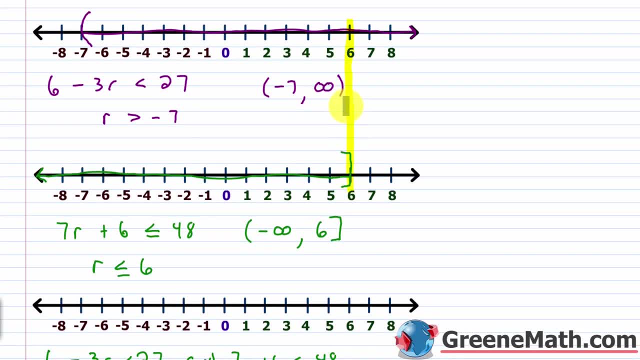 Here's 6, right here. kind of think about this as the cut off for the largest value. 6 is included because this has a bracket here and in this situation it's going this way forever and ever and ever. so 6 is included Now, with negative 7, it's not. 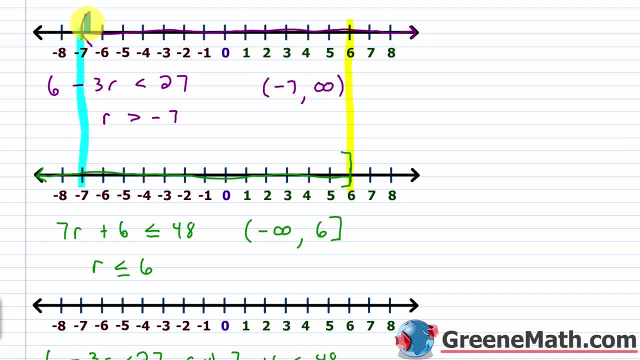 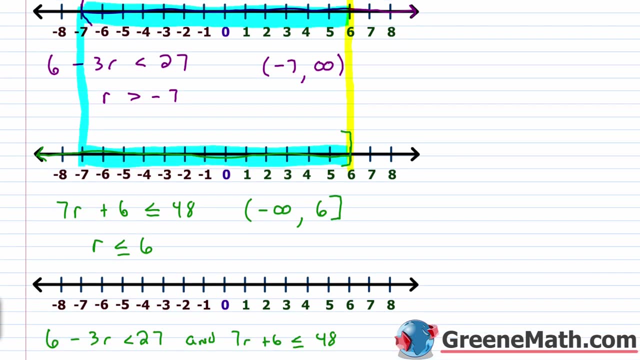 included, because in this case it's got a parenthesis there. it's not included there. So that's your cut off, anything larger than negative 7.. But kind of anything in between here. anything in between would work as a solution for each of them, So graphically. 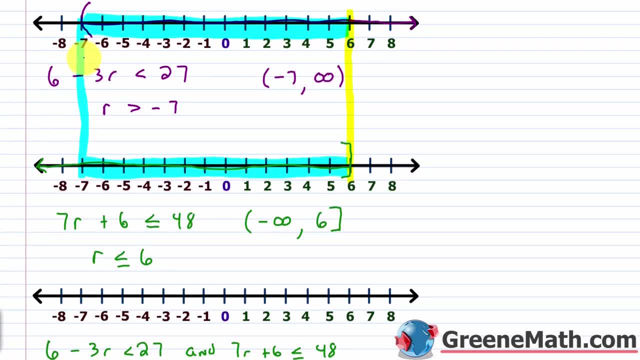 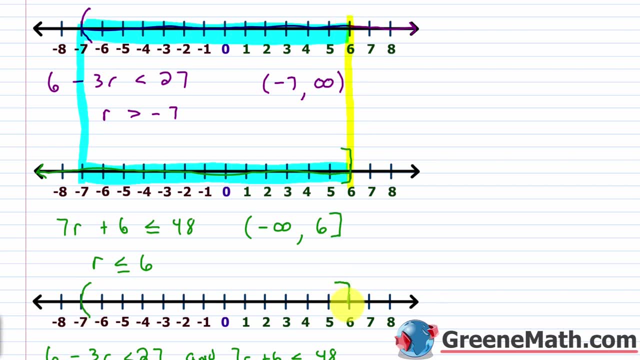 it's pretty easy to see without even referencing this. I know that at negative 7 I would have a parenthesis because it's not included. I know at 6 I would have a bracket because it is included and I would shade everything in between, Everything in between. 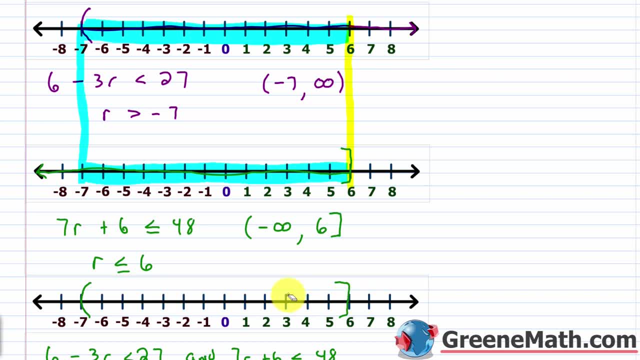 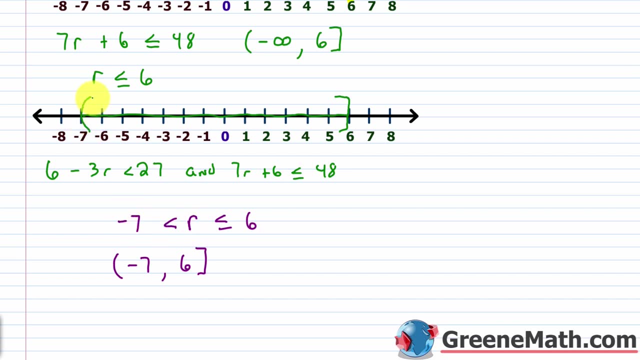 And again, the reason we're doing this is it has to be a solution to each, And this is the section of the number line that satisfies both. So, again, our solution for the compound inequality is that r is greater than negative 7, which is displayed here. it's got to be greater than negative 7. 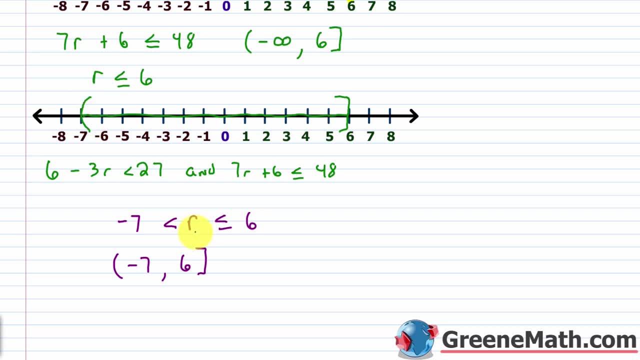 negative 7 is not included- we put a parenthesis there- and it's also less than or equal to 6. So it could be 6, which is why we have a bracket, and then anything less. So it's this range here: anything greater than negative 7. 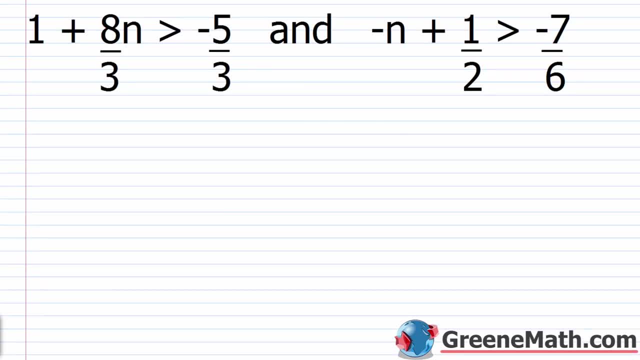 up to and including the number 6.. Alright, for the next one, we're going to work on one with some fractions involved and nothing we're not used to. so what we have here is 1 plus 8 thirds. n is greater than negative 5 thirds. 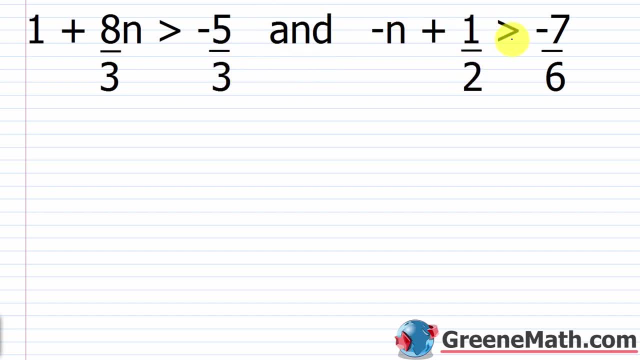 and we have negative n plus 1 half is greater than negative 7 sixths. Again, we want to solve each one separately, so I'm going to start out with 1 plus we have 8 thirds n, and this is greater than negative 5 thirds. 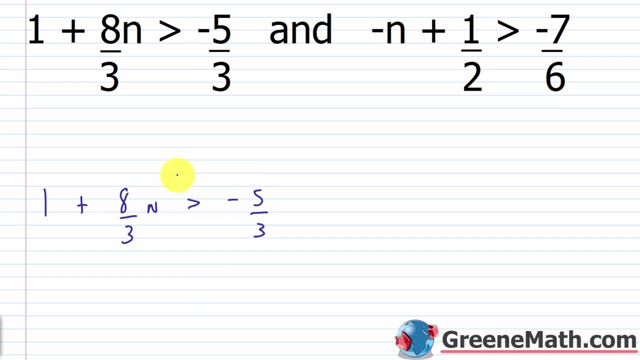 so I want to clear the denominators. so I'm going to multiply both sides here by 3, and so 3 times 1 is 3, plus 3 times 8, thirds is 8, then times n, and this is greater than 3 times negative, 5 thirds is: 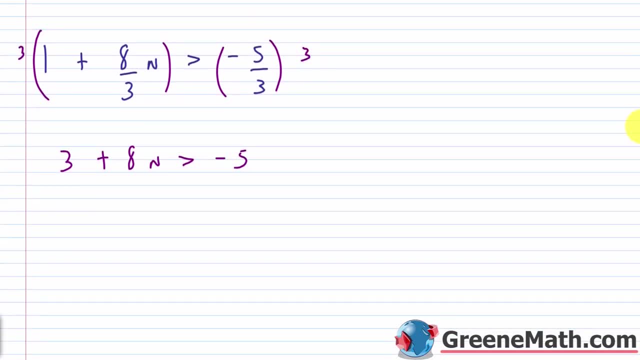 negative 5.. Let's scroll down a little bit and get a little room going. I would subtract 3 away from each side of the inequality. this will cancel. I will have 8. n is greater than negative 8. divide each side by 8 and I get. 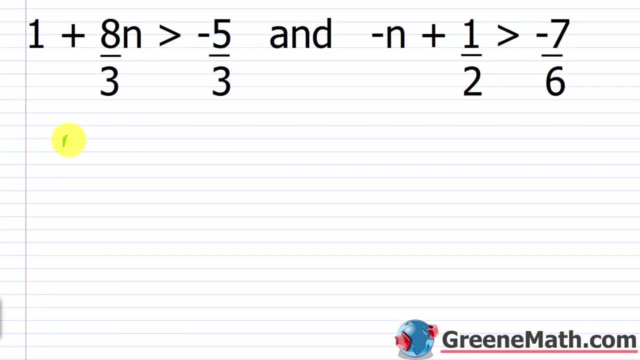 n is greater than negative 1. ok, so again, n is greater than negative 1. now over here where I have negative n, so I have negative n plus 1. half is greater than negative 7, sixths. again I want to clear the denominators, the LCD here. 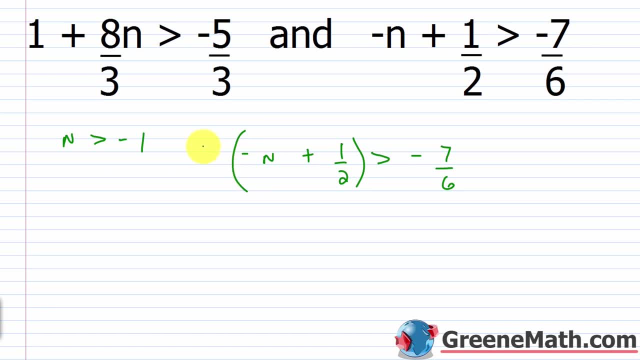 would be 6. right, I've got a 2 and a 6 LCD would be 6. so multiply both sides of the inequality by 6. 6 times negative n is negative 6 n plus 6 times 1. half is 3. 6 cancels with 2 and. 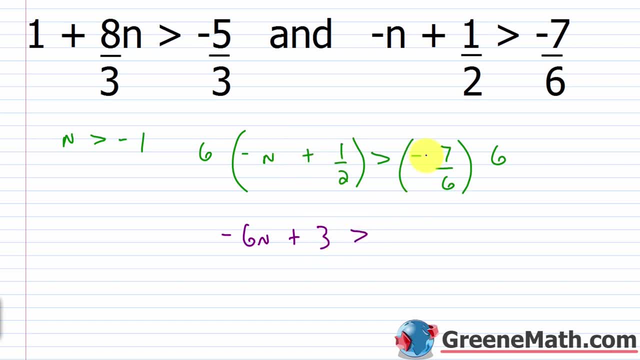 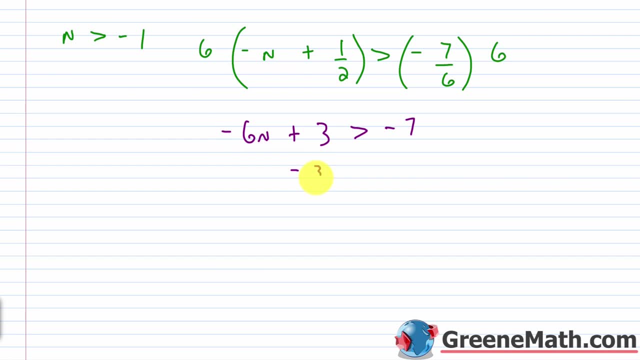 gives me 3. 3 times 1 is 3. this is greater than negative 7. 6 times 6 is negative 7. so now let me scroll down a little bit, a little room going subtract 3 away from each side. this will cancel. I will have. 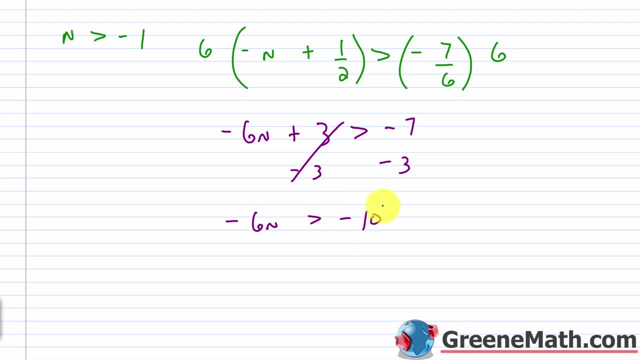 negative 6 n is greater than negative 10, we will divide each side by negative 6. remember, if I divide by a negative, I've got to flip the direction of the inequality symbol. that's a greater than, so now it's going to be a less than. 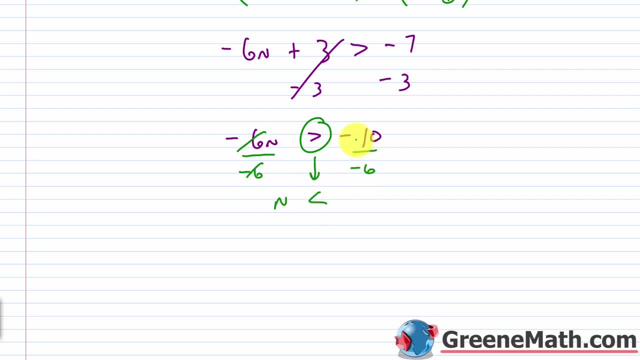 so this cancels with this and I have n. this is less than negative. 10 over negative. 6 is positive and I know each is divisible by 2. 10 divided by 2 is 5. 6 divided by 2 is 3. so this is positive 5. 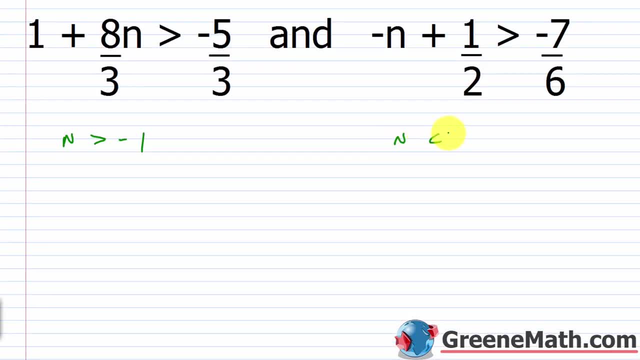 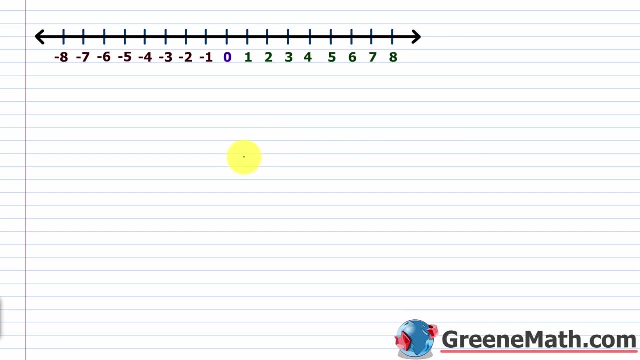 thirds. so then again, this was: n is less than 5 thirds, so we're just going to use one graph this time. we can put it together and have one solution. so we found that for 1 plus 8 thirds, n is greater than negative 5 thirds. 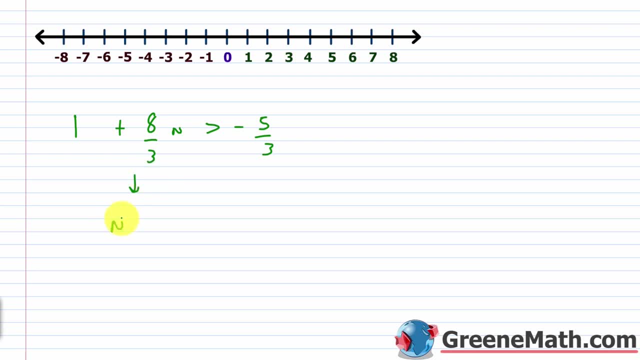 the solution was n is greater than negative 1. so in interval notation that looks like this: you have a parenthesis, a negative 1 comma, infinity, and then a parenthesis. graphically we know that at negative 1 we would have a parenthesis and then we would shade everything. 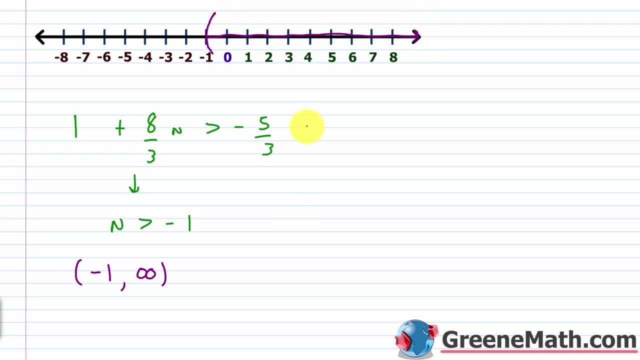 to the right. now I'm going to add something to this I have, and so we're connecting this. we have negative n plus 1. half is greater than negative 7 sixths. we found that the solution for this was n is less than 5 thirds. 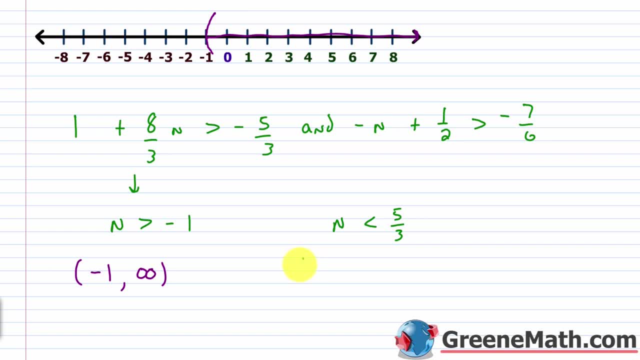 so in interval notation that looks like this: you have negative infinity next to a parenthesis comma. you'll have 5 thirds and that'll be next to a parenthesis as well, because it's not included. so, graphically, if I look at this, where's 5 thirds at? well, it's basically: 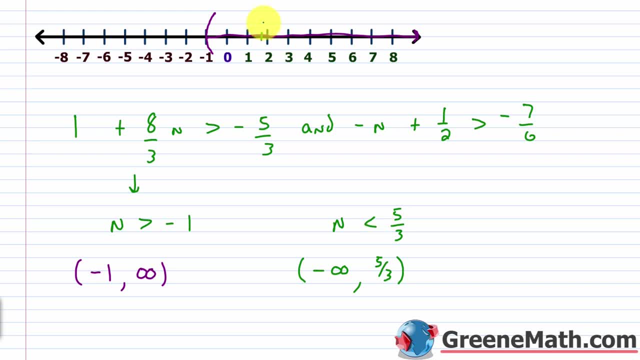 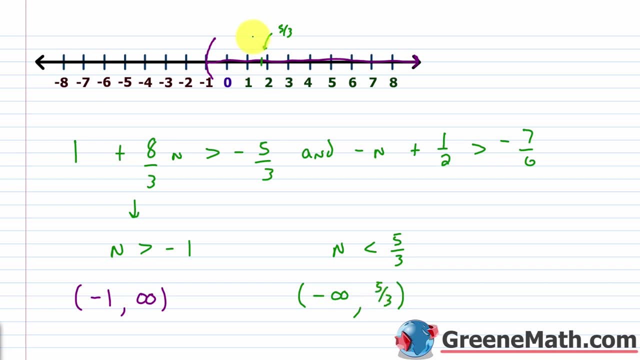 1 and 2 thirds. so it's something like: right here let's say there's no notch for it, but let's create one and say this is 5 thirds. so what I'd be doing is I'd be placing a parenthesis there, placing to the left. 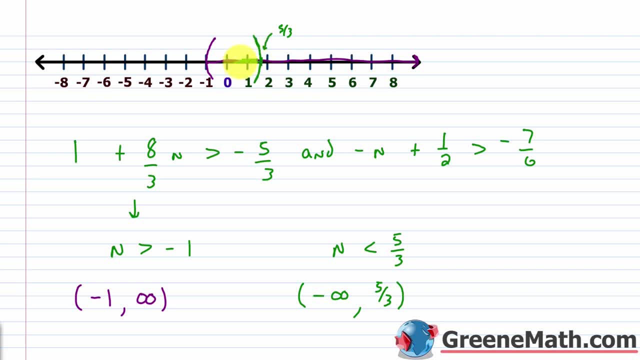 okay, and then I would shade everything. going this way, right, going this way, it's easy to see graphically what the intersection would be: it would not include negative 1, it would not include 5 thirds, but it would include everything in between. so let me erase. 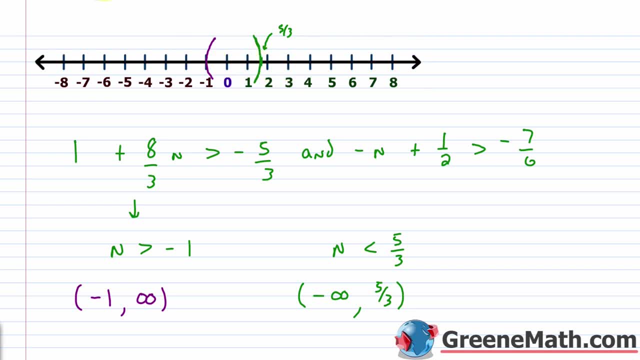 all of this and I'll keep those two parenthesis there and I want to shade everything in between. this is my solution for the compound inequality and I could also write it with n in between. so I could write n in between, and we know that it's greater. 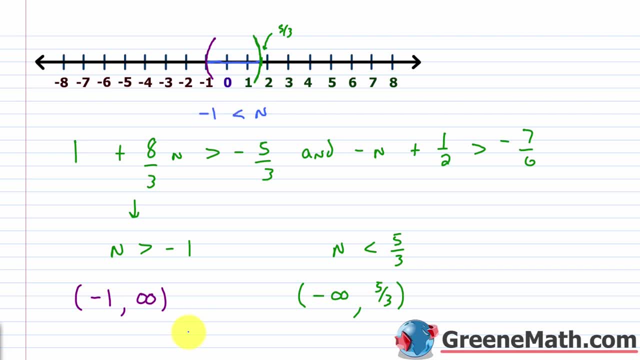 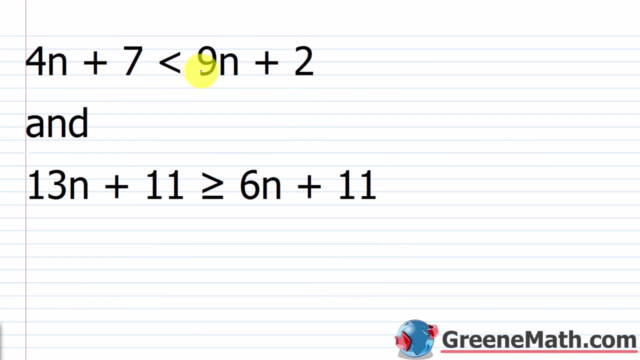 than negative 1 and it's less than 5 thirds. alright, let's take a look at another one. so we have: 4n plus 7 is less than 9n plus 2, and 13n plus 11 is greater than or equal to. 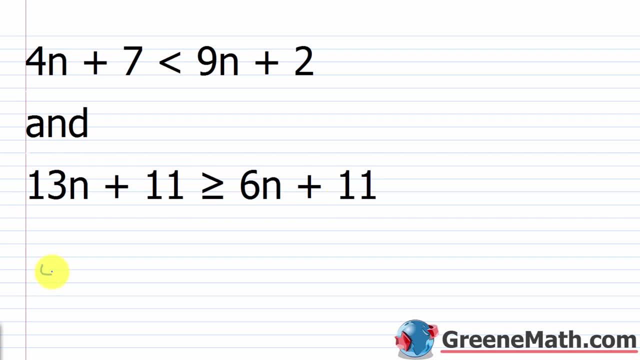 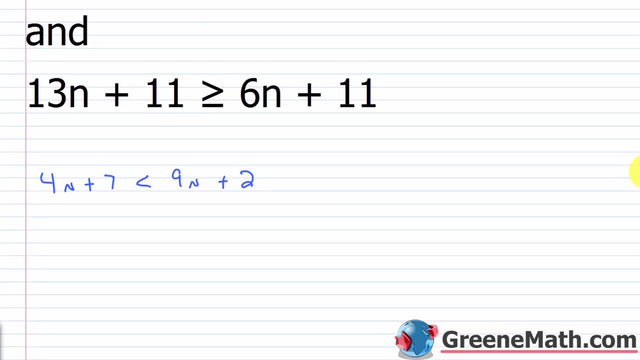 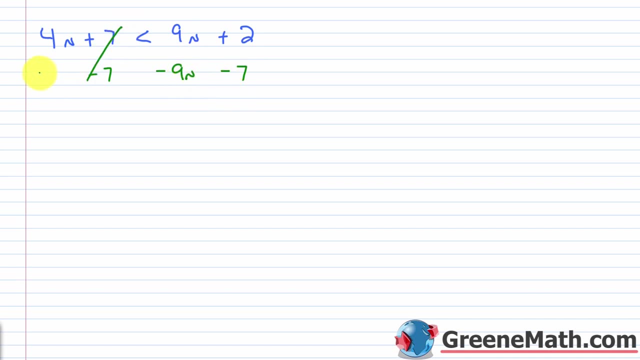 6n plus 11. so let's start out with this one we have. 4n plus 7 is less than 9n plus 2. let's solve that guy. so I want to subtract 7 from each side. that'll cancel. I also want to subtract 9n from each side. 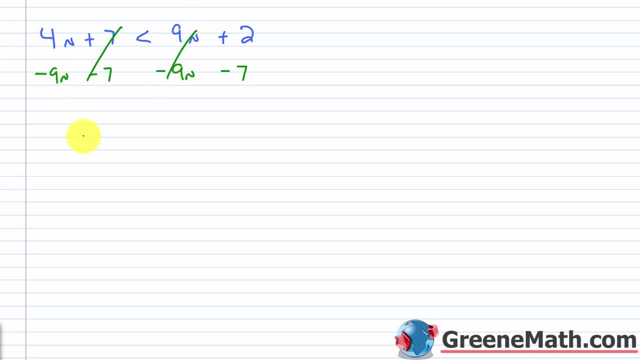 that'll cancel. 4n minus 9n is negative 5n. this is less than 2 minus 7 is negative 5. we divide each side by negative 5 and don't forget to flip this. so right now that's a less than. 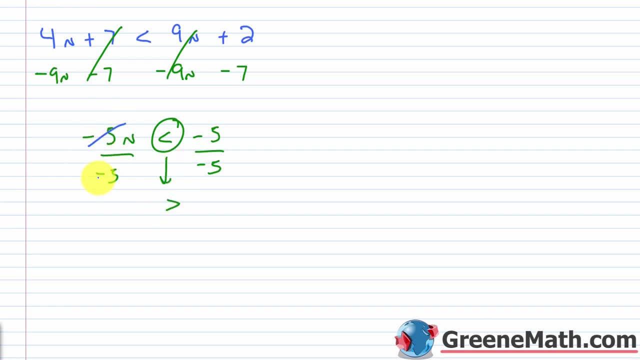 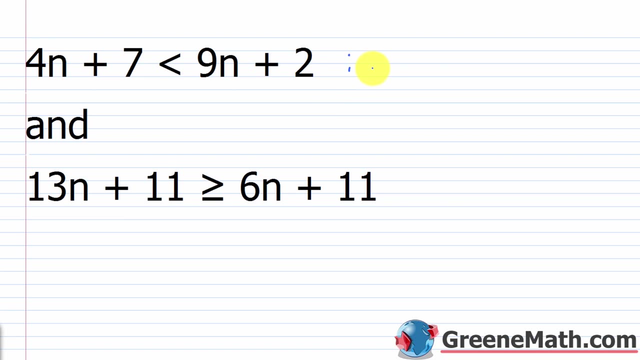 it's going to become a greater than- and this would cancel with this and give me n. so n is greater than negative 5 over negative 5 is 1. so for this one we can say that n is greater than 1. for the next one, 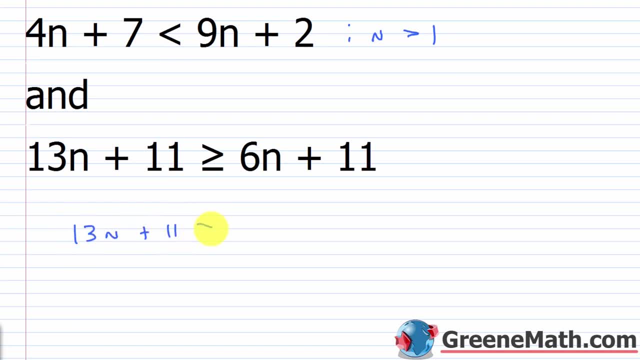 we have 13n plus 11 is greater than or equal to 6n plus 11. I know if I have the same thing on each side of an inequality or an equation, I can just get rid of it because I can subtract 11 away from each side. 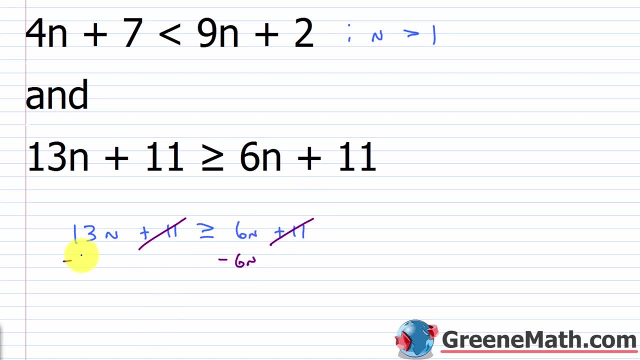 and now I can just subtract 6n away from each side, so I'll have 13n minus 6n, that's 7n is greater than or equal to. this has all been cancelled, so it's 0 now. I divide both sides by: 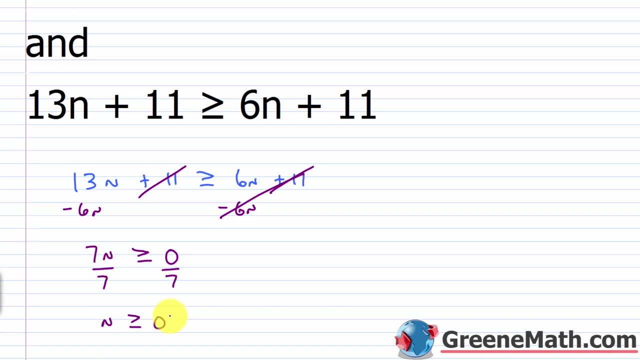 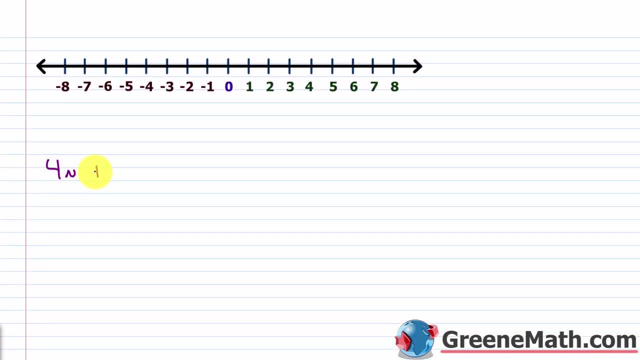 7 and I get: n is greater than or equal to 0. so this is: n is greater than or equal to 0. so again we had: 4n plus 7 is less than 9n plus 2 and 13n- 13n. 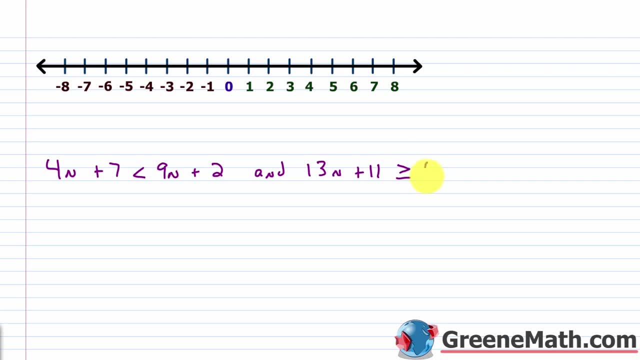 plus 11 is greater than or equal to 6n plus 11. so the solution for this guy was that n is greater than 1. or we could say in interval notation you'd have a parenthesis, a, 1, an infinity symbol and a parenthesis. graphically I would put a parenthesis. 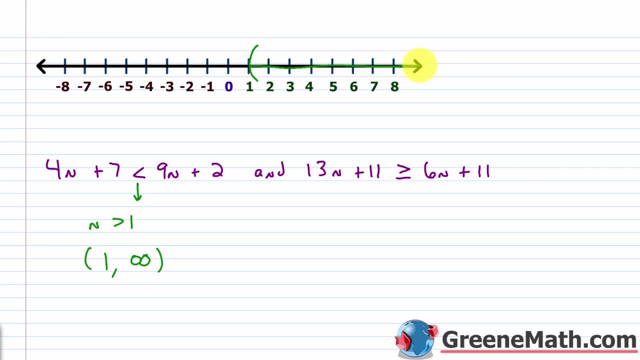 at 1 and I'd shade everything to the right now for this guy, 13n plus 11 is greater than or equal to 6n plus 11. we found that n was greater than or equal to 0, so in interval notation you'd have a bracket next to 0. 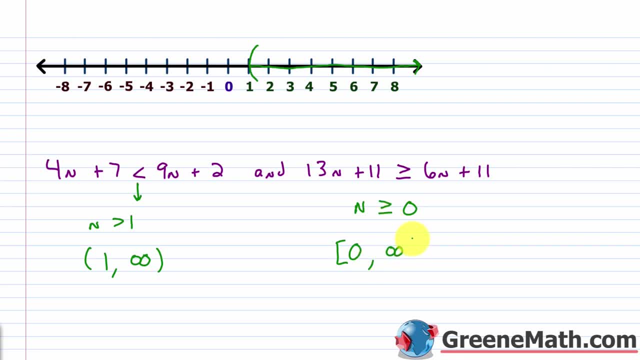 because 0 is included, comma and then infinity, and you always use a parenthesis there. now for this one, I'm going to have a bracket that starts at 0 and I'm going to shade everything to the right, so it's pretty easy to see what the solution for the 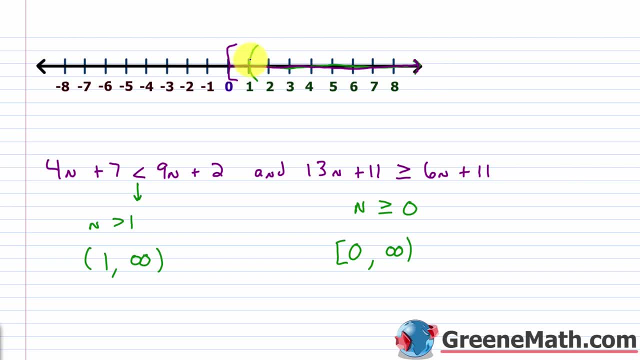 compound inequality is anything to the left of 1 and also including 1 doesn't work, because it has to work for both, and it would not be a solution for this original, because here n has to be greater than 1, but anything that's larger than 1 works for. 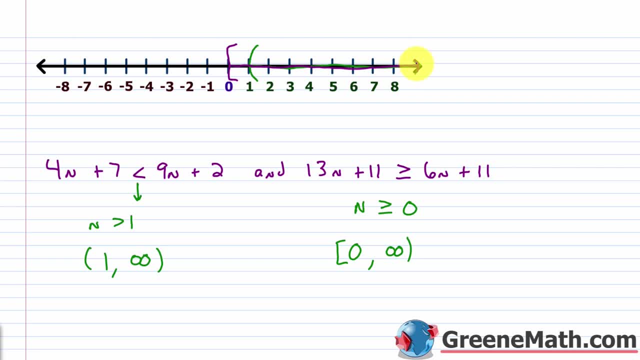 both because both areas are shaded there. and so for the compound inequality- let me just erase this part- it would essentially be the solution for this guy. so it would be: n is greater than 1. so the solution for the compound inequality is that n is greater than 1. 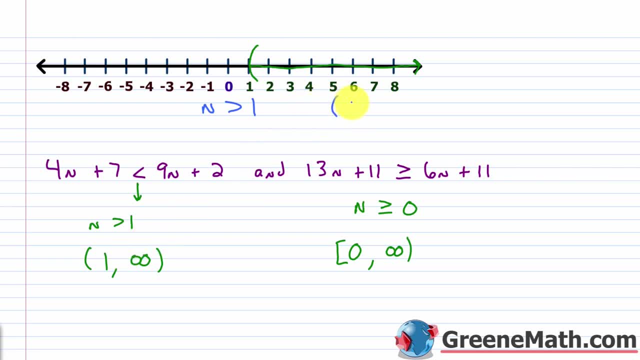 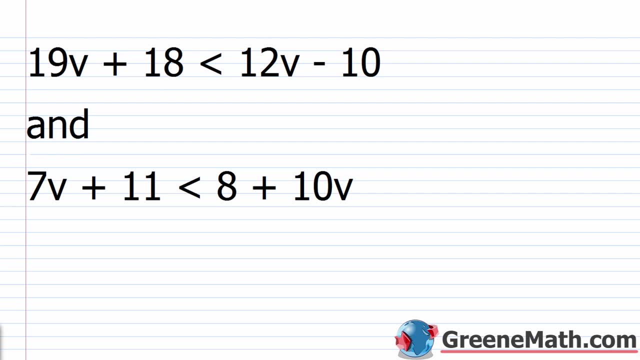 for an interval notation. again the same thing as this: 1 is not included, but anything larger is alright. let's take a look at one more with and, and then we'll start talking about the scenario of: or. so we have 19v plus 18 is less. 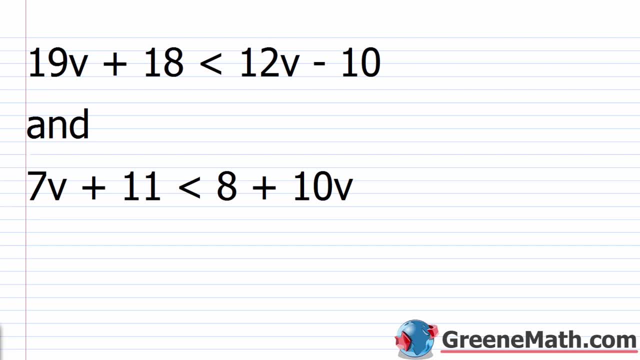 than 12v minus 10, and 7v plus 11 is less than 8 plus 10v. so if I start with this first one here, 19v plus 18 is less than 12v minus 10. so I'm going to. 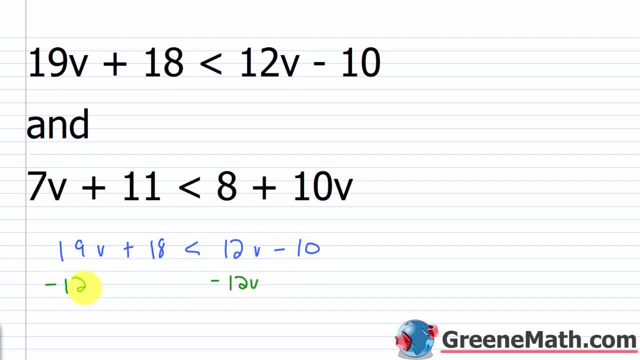 subtract 12v away from each side, that's going to cancel. I'm going to subtract 18 away from each side. that'll cancel. 19v minus 12v is going to give me 7v and this is less than negative 10 minus. 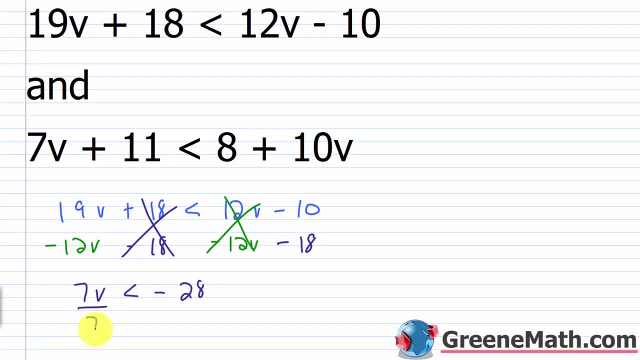 18 is negative 28. divide each side by 7 and we'll get that v is less than negative 4. so this is v is less than negative 4. alright, for the second part of this, I have that 7v plus 11 is less. 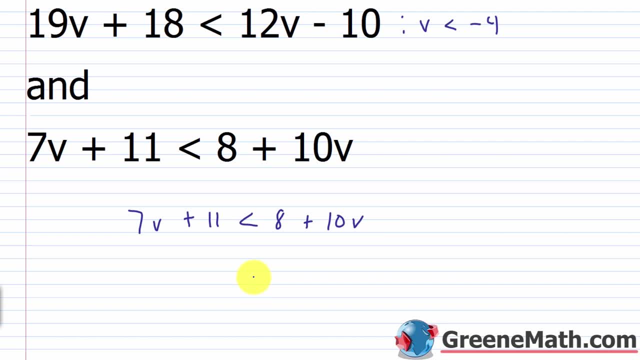 than 8 plus 10v again. what I can do is subtract 10v away from each side. that's going to cancel. 7v minus 10v would give me negative 3v. I would subtract 11 away from each side. that's going to cancel. 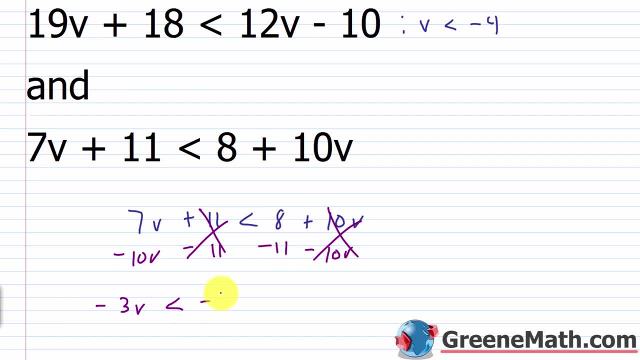 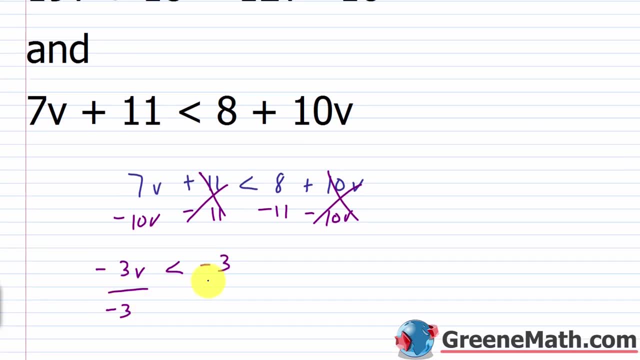 so negative 3v is less than 8 minus 11 is negative 3. I will let me scroll down and get a little room going. I will divide both sides by negative 3. remember I'm dividing by a negative, so I've got to flip the direction. 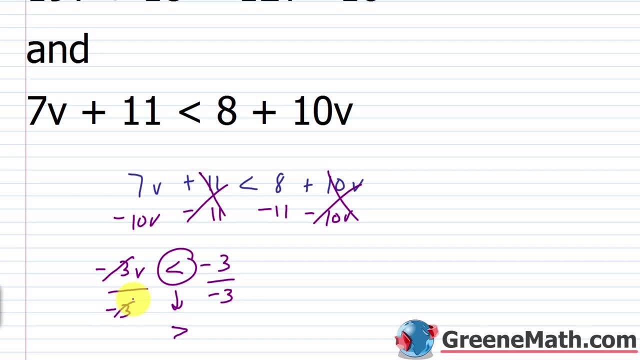 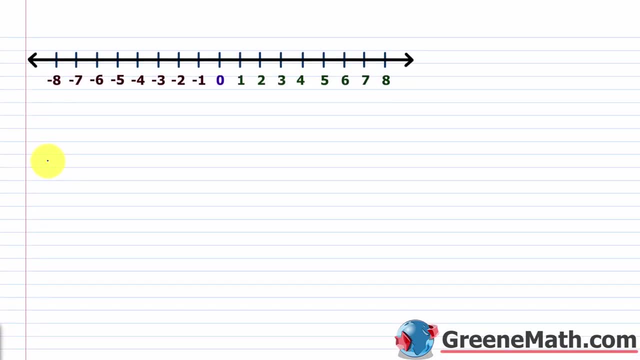 here, so this becomes a greater than so this cancels with this. I have: v is greater than 1, so this is v is greater than 1, and again our problem is: 19v plus 18 is less than 12v minus 10, and 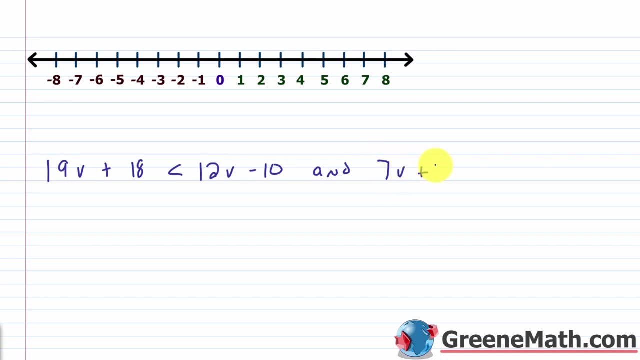 7v plus 11 is less than 8 plus 10v. now the solution for this guy right here, we know, is v is less than negative 4. so in interval notation we would say that we have a parenthesis next to negative infinity, because anything less than negative 4. 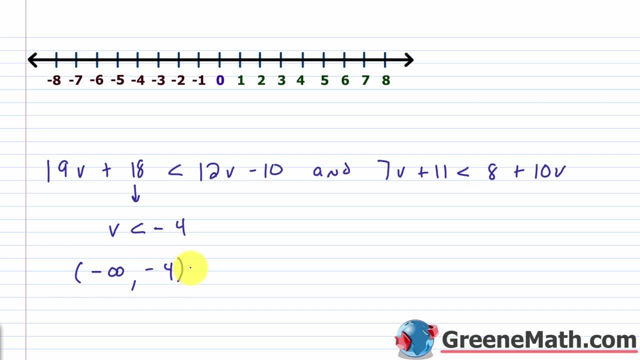 so up to, but not including, negative 4. so that's a parenthesis next to that. graphically, at negative 4 I put a parenthesis facing to the left and I would shade everything going this way and for this guy over here. we found that v was greater. 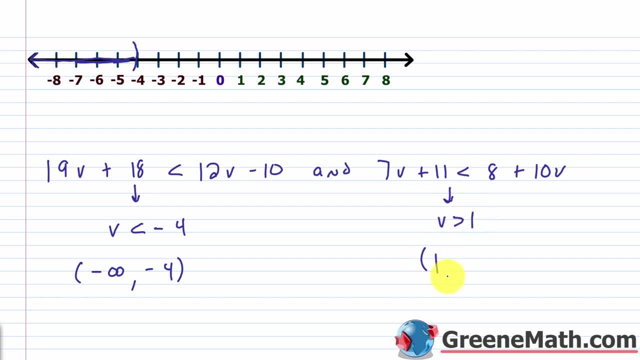 than 1. so in interval notation I put a 1. it's not included, so I have a parenthesis there. then comma: I have the infinity symbol, parenthesis next to that. graphically I'd find 1, I'd put a parenthesis there and I'd shade everything to the right. 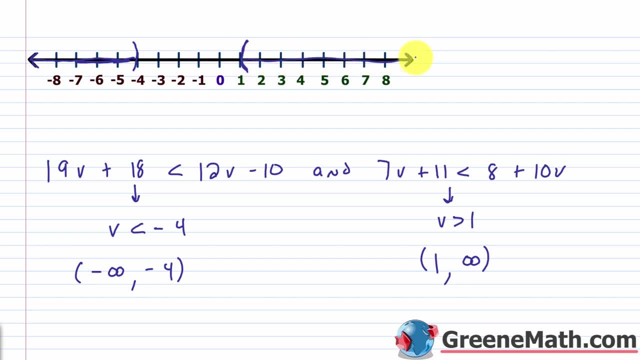 do you see a problem with this scenario? there's a solution for each part of the compound inequality, but the compound inequality itself has no solution. why is that the case? because it has to overlap. it has to be a solution for each, and that doesn't exist. there's no solution here. 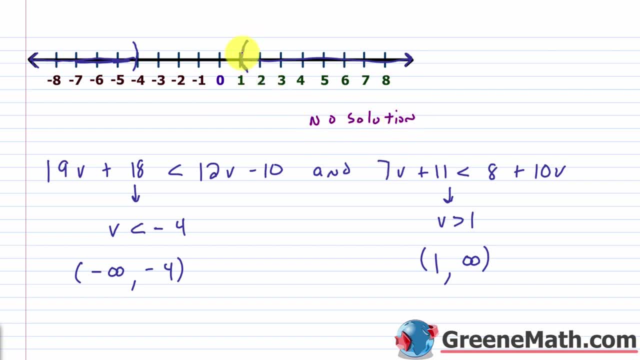 no solution because if you look here, for this guy right here, this 7v plus 11 is less than 8 plus 10v. that's satisfied by numbers that are greater than 1. this guy right here, this 19v plus 18, is less than 12v minus. 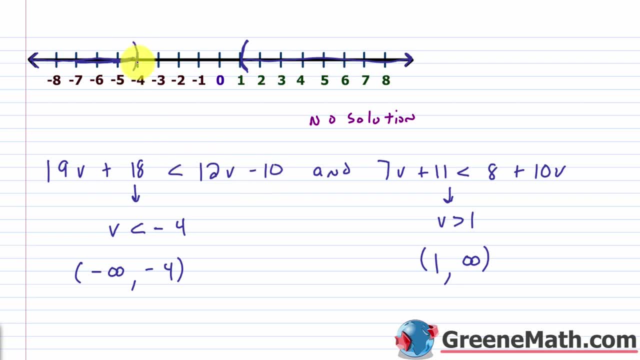 10 that's satisfied by numbers that are less than negative 4. so there is no number that is less than negative 4 and also greater than 1. that doesn't exist, and so there is no solution. now, one thing that your teacher might want you to do. remember, you have a symbol. 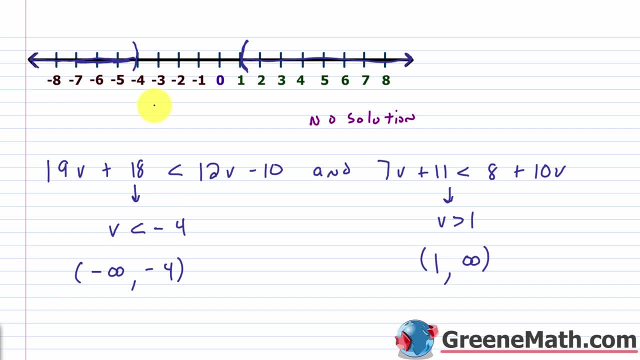 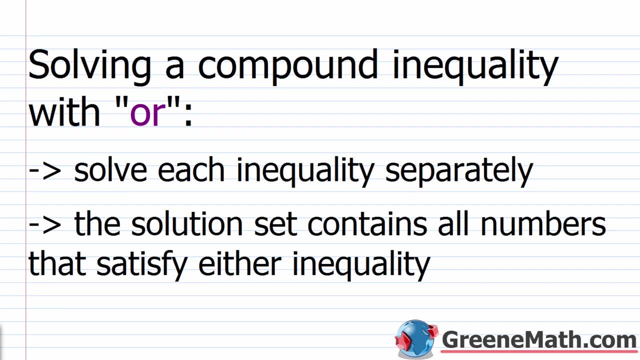 when you have a set that contains no elements. it's a symbol for the null or empty sets. you might just want to put no solution and then put this symbol if you get this scenario, alright. now let's talk about solving a compound inequality with the word or so again you want to. 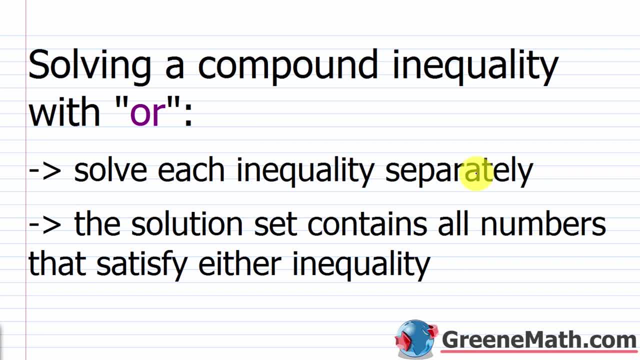 solve each inequality separately, so you always do that part. the next part is a little bit easier. actually, you just say the solution set contains all numbers that satisfy either inequality- so it doesn't matter if it's a solution to only one of them- or it could be a solution to both. 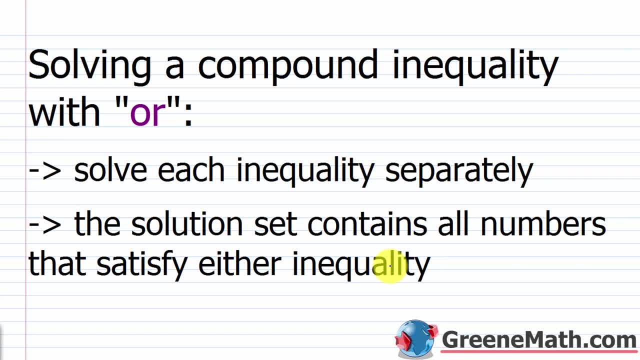 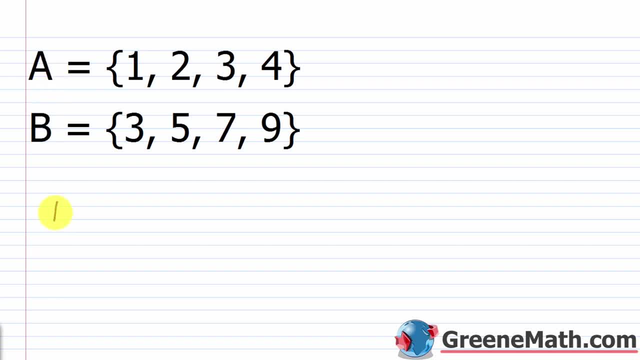 either way, it's going to be a solution for the compound inequality. so, as an example, with sets, I go back to my set A and set B if I want the union of these two sets. so the union of A and B is equal to what? well, everything. 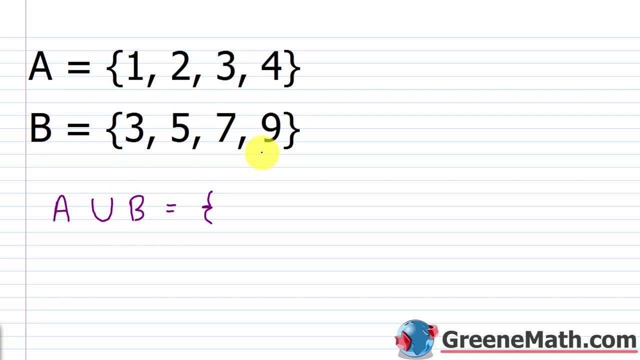 goes in. the only thing you gotta make sure of is, if you have an element that's common to both, you list it only once. ok, only once. so you have 1,, 2, 3 only gets listed once, then 4, then 5, then 7. 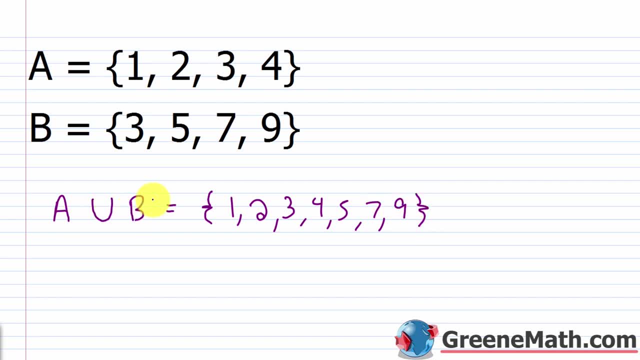 then 9, so the union of these two sets is all the elements combined. again, nothing gets double listed. so each and every element from A along with every element from B is an element of this set. alright, so let's look at the first problem we have: 5k plus 2 is greater than 32. 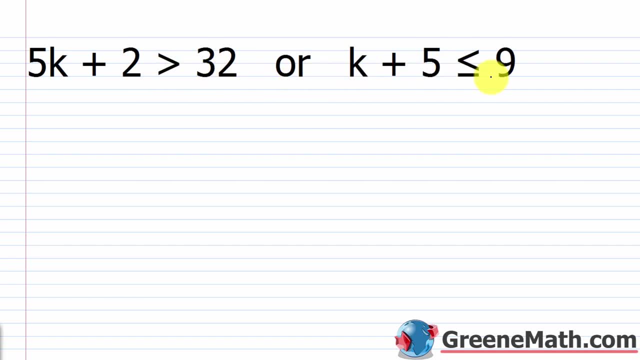 or k plus 5 is less than or equal to 9, so I want to subtract 2 away from each side over here. I'll have: 5k is greater than 30. I'll divide each side by 5 and I'll get: k is greater than 6. 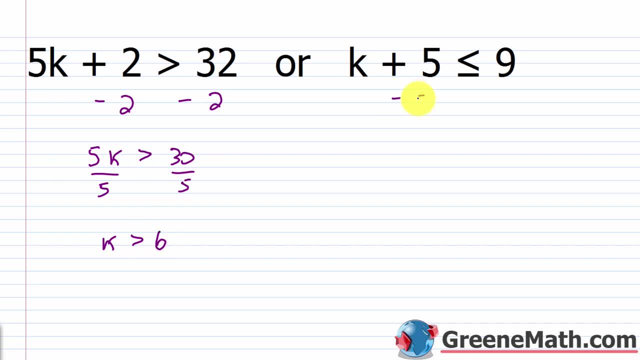 so then we have, or so we have this one over here. subtract 5 away from each side, I'll have: k is less than or equal to 4, so again we have 5k plus 2 is greater than 32, or we have k plus. 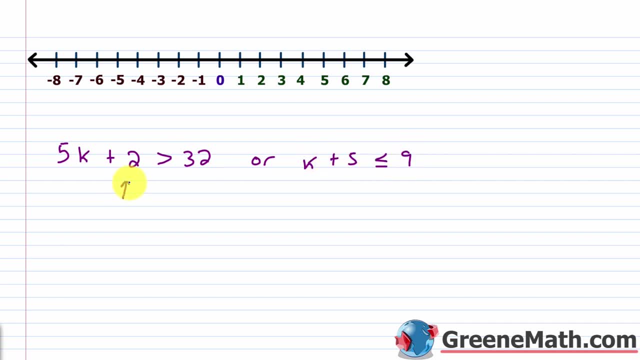 5 is less than or equal to 9. so for this guy we found that k was greater than 6. in an interval notation that looks like this: you have 6 comma infinity with a parenthesis at each end. graphically I'd put a parenthesis at 6 that faces to the right. 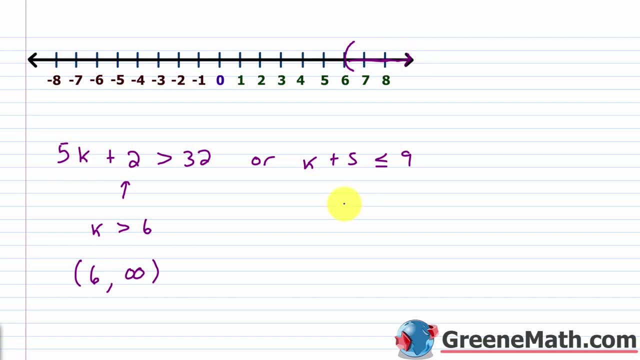 and I'd shade everything to the right. then, for k plus 5 is less than or equal to 9. we found that k was less than or equal to 4, so in an interval notation I'd have a negative infinity comma, a, 4, with a bracket next to 4. 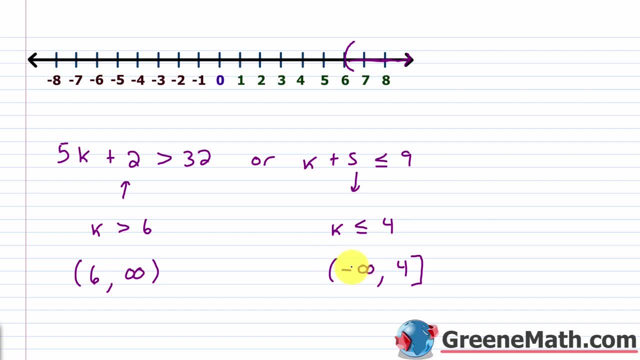 and a parenthesis next to negative infinity. so I'd find 4, I'd put a bracket facing to the left, because anything less than- and I'd shade all of this to the left. now we just saw that if we had the connective word, and we don't have a solution, 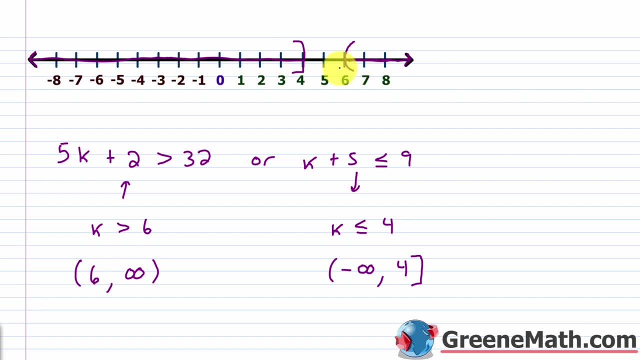 because nothing is going to overlap. there's no intersection between the two solution sets, but with or it's different. it can be a solution to this guy or this guy. it's a solution for the compound inequality. so our solution set is written like this. we would say that: 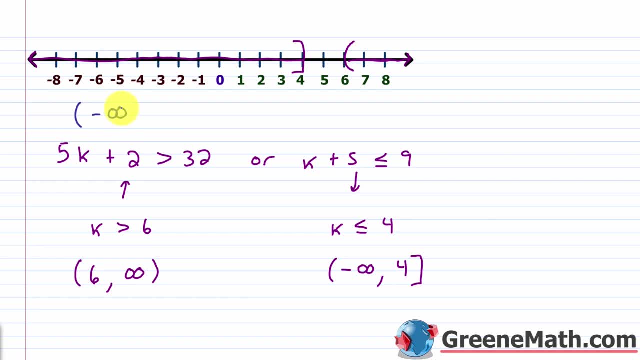 we have this set, so negative infinity up to and including 4. it's the union of this. I'm going to put the union symbol with this guy. so anything greater than 6 out to infinity. so it's the union of the two sets and, graphically, 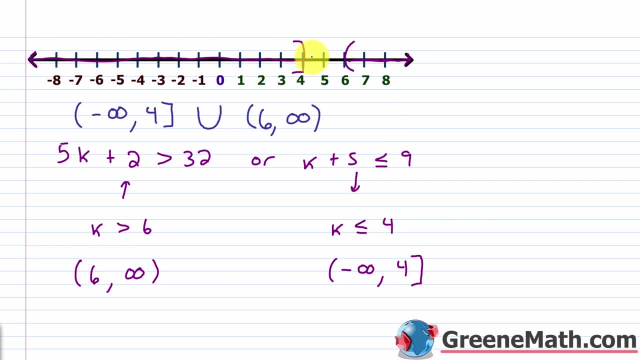 I don't need to do anything else. it's 4 or anything less. so that's all part of the solution, and then anything greater than 6. so here's your solution using interval notation, and here it is graphically, and then, additionally, you could write it just saying that: 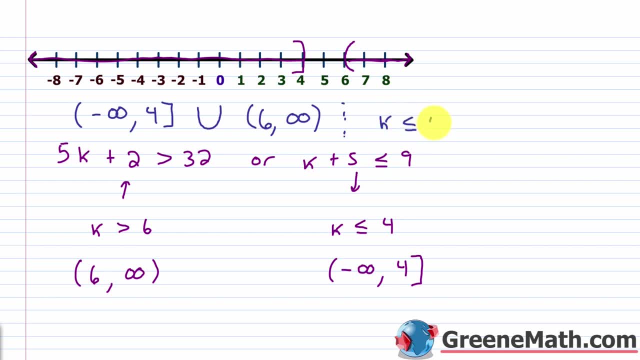 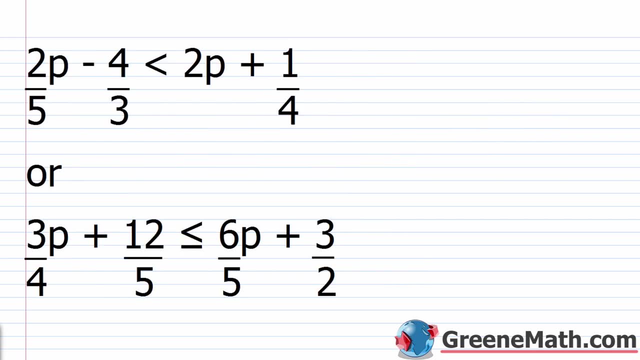 k is less than, or equal to 4, or just put the word or k is greater than 6. alright, for the next one we're looking at: 2 fifths p minus 4 thirds is less than 2p plus 1 fourth, or 3 fourths p. 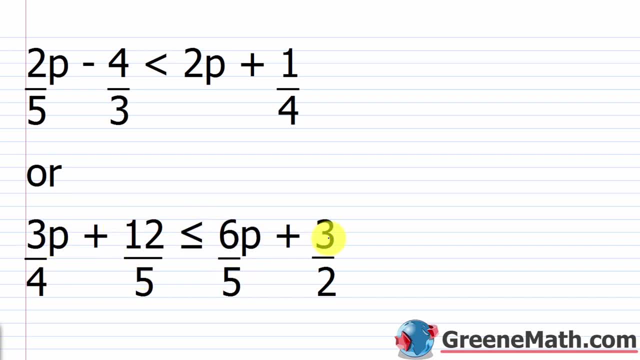 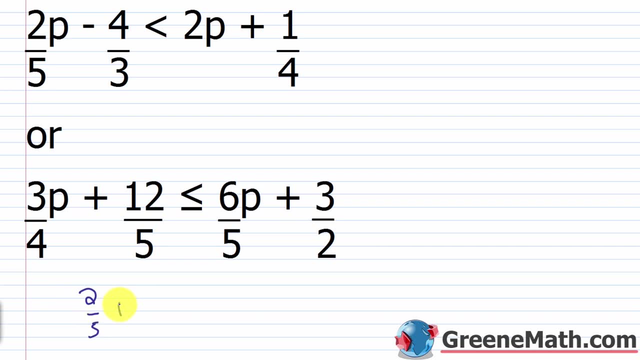 plus 12 fifths is less than or equal to 6 fifths p plus 3 halves. alright, so let's start out with this guy right here. so I have 2 fifths p minus 4 thirds is less than 2p plus 1 fourth. 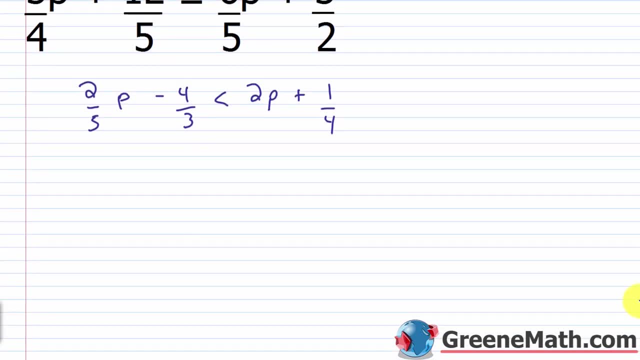 so I want to clear my denominators and the LCD here would be 4 times, 3 times 5 or 60. so let me multiply both sides by 60, 60 times 2. fifths 60 would cancel with 5 and give me 12. 12 times 2 is. 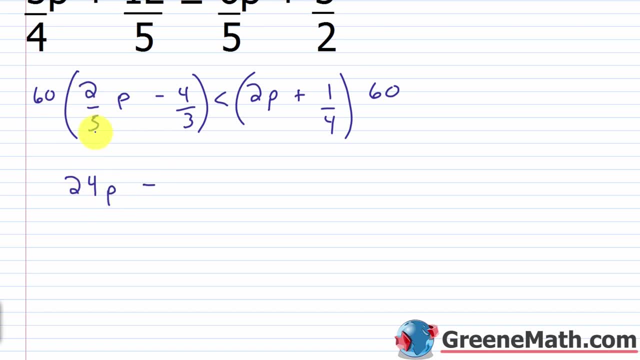 24. so this would be 24p, then minus 60 times 4 thirds. 60 divided by 3 is 20. 20 times 4 is 80. this is less than 60 times 2p is 120p, then plus 60 times. 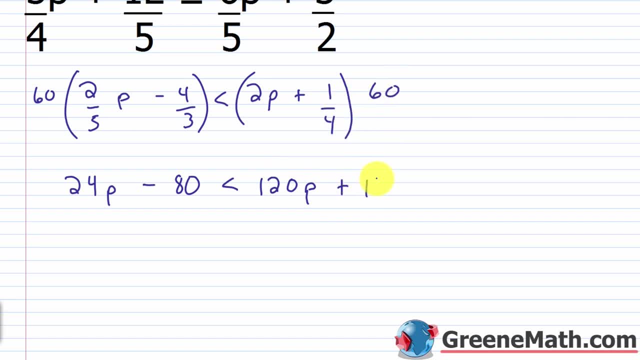 1. fourth, 60 divided by 4 is 15. 15 times 1 is 15. so then what I can do is add 80 to each side and I can subtract 120p from each side. this is going to cancel and this is going to. 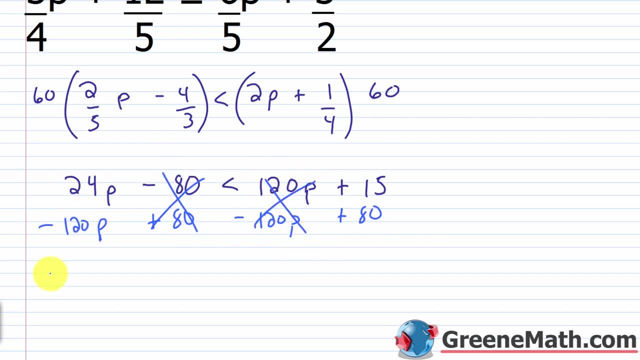 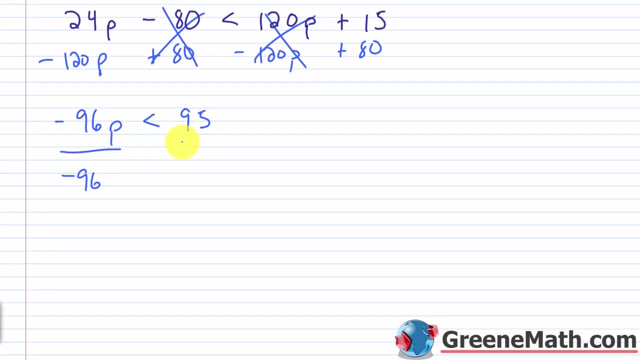 cancel. 24 minus 120 is negative 96. so this would be negative 96p. then it's less than 15 plus 80 is 95. so if I divide both sides by negative 96- remember I've got to flip the direction of this guy- 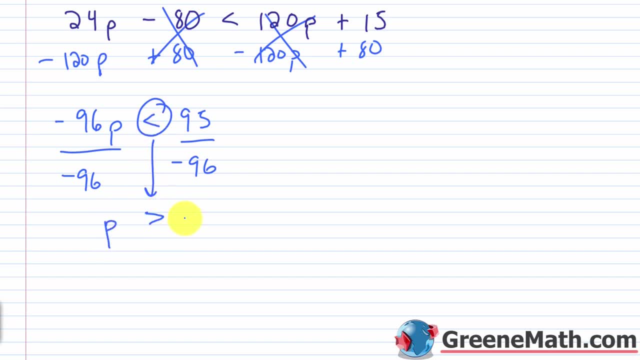 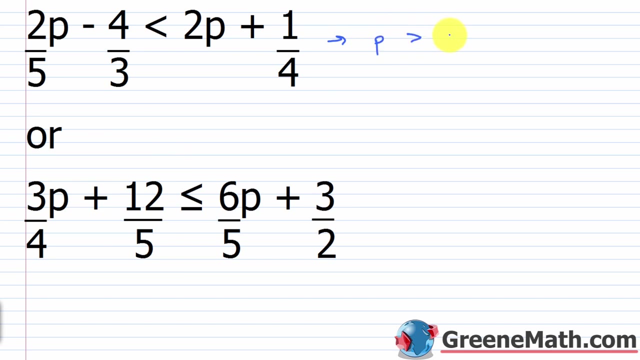 this becomes a greater than now I'll have. p is greater than 95 over 96 and because this is negative here, I'll put a negative out in front. so p is greater than negative 95 over 96. so p is greater than negative 95 over. 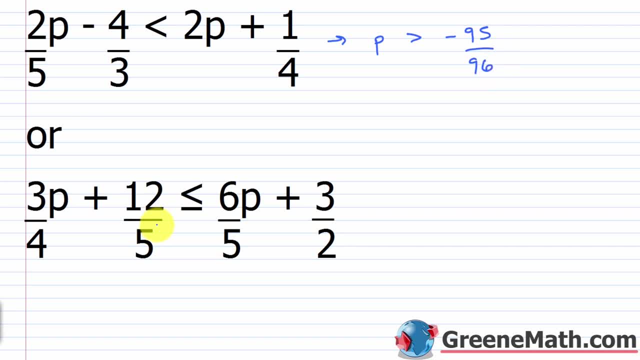 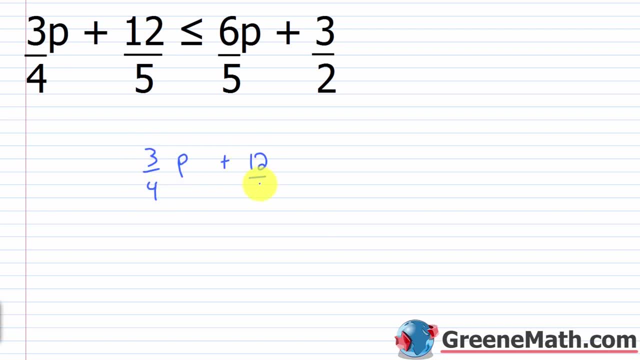 96. now we'll deal with this one, so let's scroll down a little bit. so I have 3 fourths p plus 12. fifths is less than or equal to 6 fifths p plus 3 halves, so the LCD here would be what we have: 2. 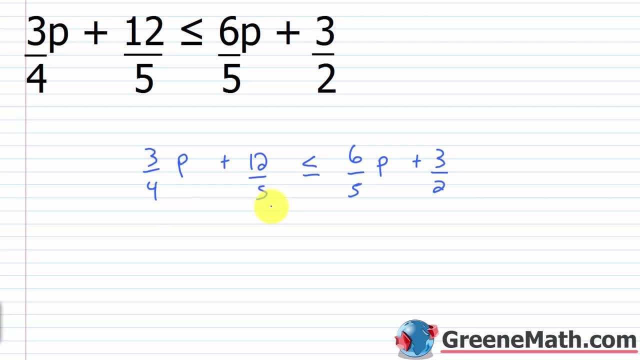 4- 5. so basically it would be 4 times 5 or 20. we'll multiply both sides by 20, and so 20 times 3, fourths 20 would cancel with 4 and give me 5, 5 times 3 is 15. 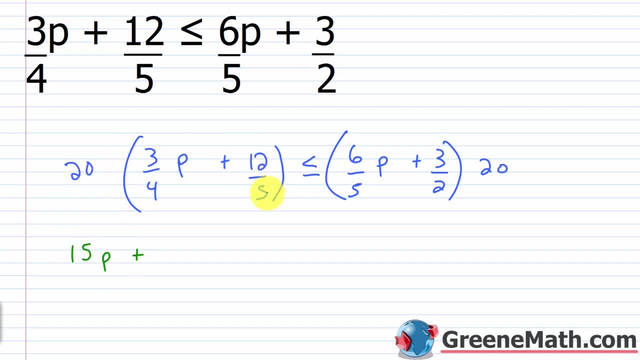 so this is 15p plus 20 times 12. fifths 20 would cancel with 5 and give me 4. 5 times 12 is 48. this is less than or equal to 20 times 6. fifths p 20 would cancel with 5 and give me 4. 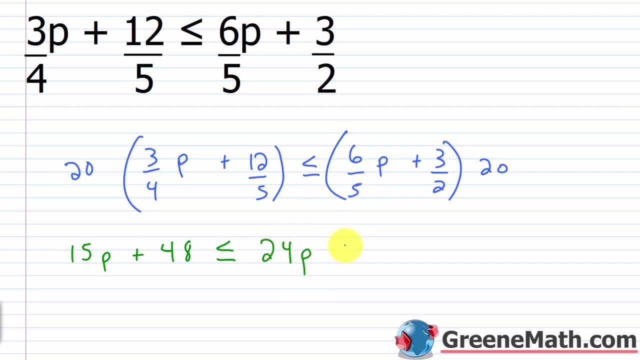 4 times 6 is 24. then times p, then plus 20 times 3, halves 20, would cancel with 2 and give me 10. 10 times 3 is 30. alright, so we can now subtract 24p away from each. 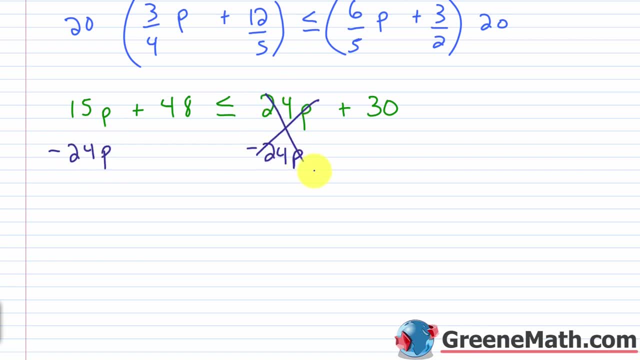 side. cancel this. you can subtract 48 away from each side. cancel this. 15p minus 24p is negative 9p, and this is less than or equal to 30 minus 48 is negative 18. we divide each side by negative 9 and again we've got to. 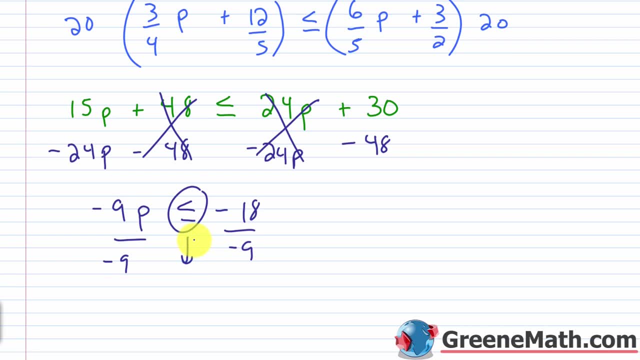 flip the direction of the inequality symbol so this becomes a greater than or equal to, so this cancels. we have: p is greater than or equal to negative 18 over negative 9 is 2, so p is greater than or equal to 2. so again, I had 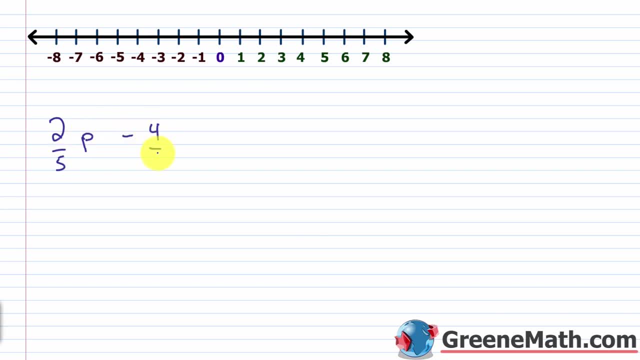 2 fifths p minus 4 thirds is less than 2p plus 1 fourth, or the other one was 3 fourths times p plus 12 fifths is less than or equal to 6 fifths p plus 3 halves. now for this. 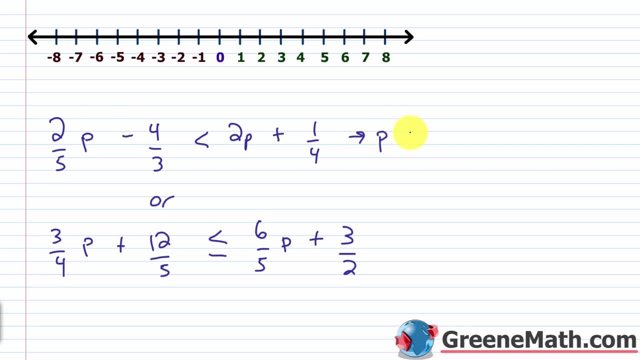 guy right here. we found that p. we found that p was greater than negative 95 over 96. so in interval notation that looks like this: we would have a parenthesis, then negative 95 over 96 and then out to infinity. of course you use a parenthesis with that as well. 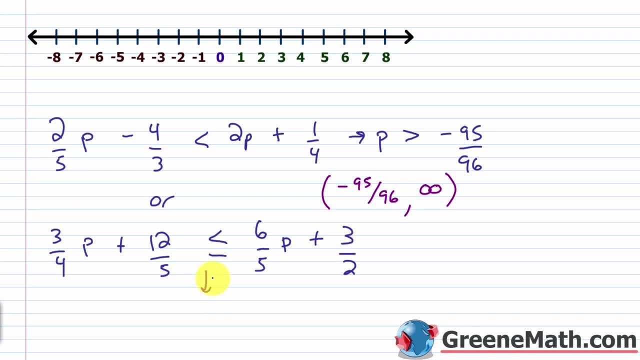 for this guy. we found that the solution was: p is greater than or equal to 2. so in interval notation you have a bracket and then you have 2 and then out to infinity. so you put a parenthesis there. graphically you can think about this one right here: negative. 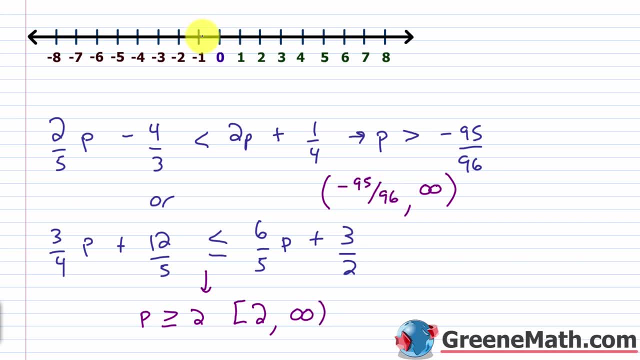 95 over 96. that's going to be a little bit to the right of negative 1, because it's not quite negative 1, it's a little bit larger, it's a little bit to the right of it. okay, if I had negative 96 over. 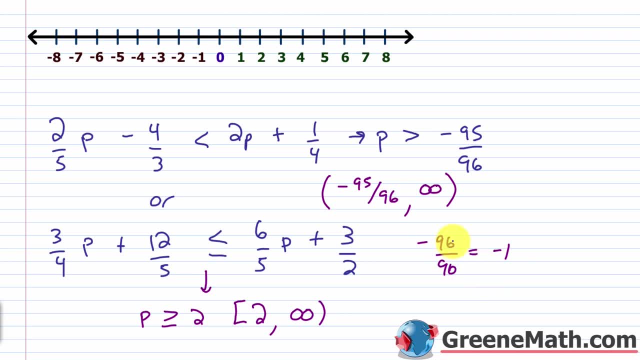 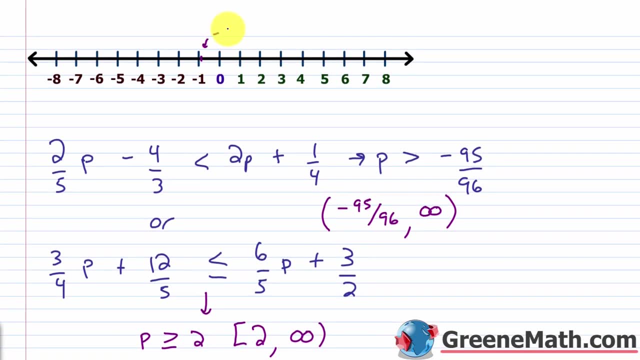 96, that equals negative 1. this is a little bit shy of that, so let's just put that right here. let's say this is negative 95 over 96 and it's anything larger than that, but not including that. so I'd put a parenthesis. facing to the right. 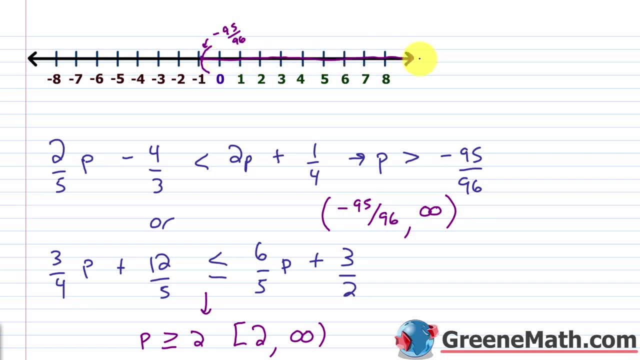 and I'd shade all of this now. the other guy was anything greater than or equal to 2, so that would be right here and I would shade everything to the right now for the compound inequality. it could be a solution either, so we would go with this solution, right here. 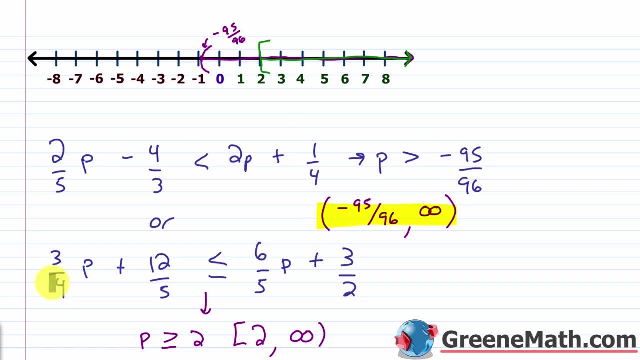 because it encompasses both. it encompasses this one and this one. so I can erase this part right here and just say that- and I can shade this in any color I want, let's just do red. this is the solution for the compound inequality and for this inequality. so the solution for 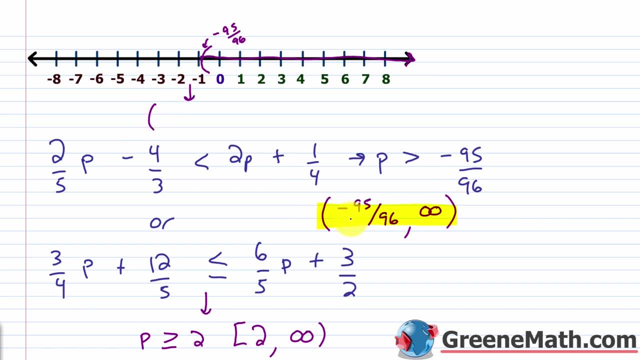 the compound. inequality is just this guy right here we'll put a parenthesis, negative 95 over 96, comma, infinity. another parenthesis. this is graphically, and then we can also just say: it's p is greater than negative 95 over 96, because this solution contains: 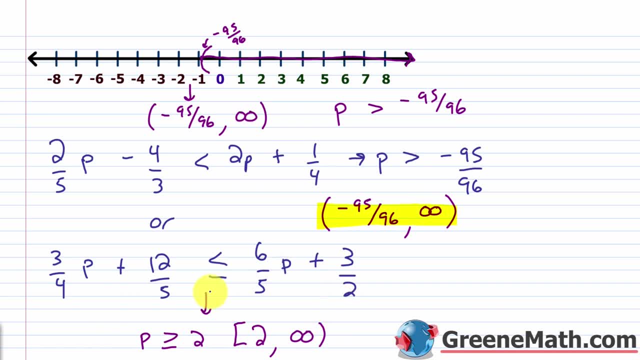 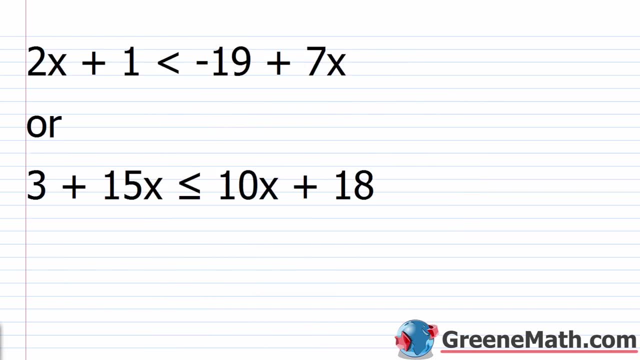 completely this solution and again, if it's a solution to, either it's a solution for the compound inequality with or. let's take a look at one final problem. so we have: 2x plus 1 is less than negative, 19 plus 7x or 3 plus 15x. 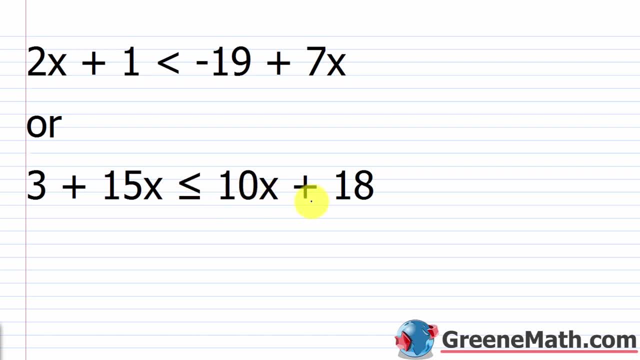 is less than or equal to 10x plus 18. so let me solve this first guy up here. so we have: 2x plus 1 is less than negative 19 plus 7x. what I want to do is I want to subtract 1 away from each. 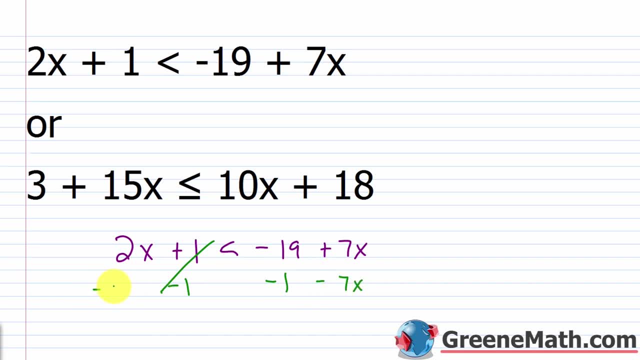 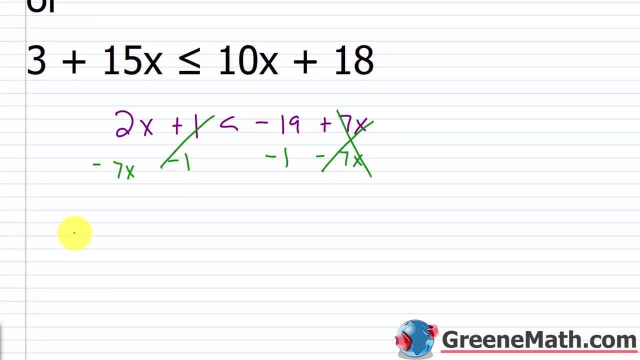 side and I want to subtract 7x away from each side, so that's going to cancel. let me scroll down and get a little room going. so 2x minus 7x is negative. 5x- this is less than negative. 19 minus 1 is negative. 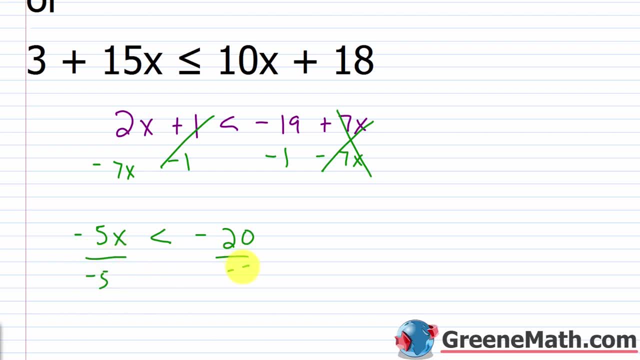 20. divide each side by negative 5, again flip the direction of this guy. so that's now greater than this. cancels with this and I'll have: x is greater than negative. 20 over negative 5 is 4. so here x is greater than 4. alright for this. 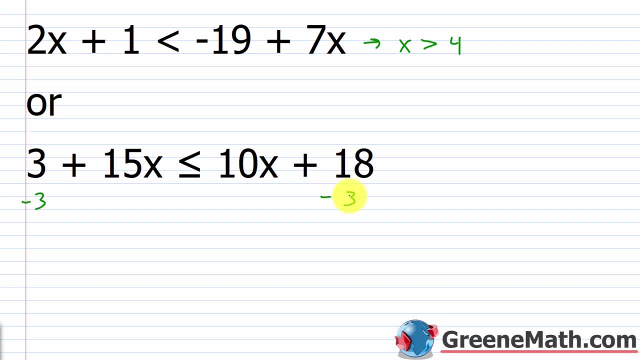 guy right here. I could subtract 3 away from each side, so that would cancel. and I could subtract 10x away from each side, so that would cancel. 15x minus 10x is 5x, and this is less than or equal to 18 minus 3. 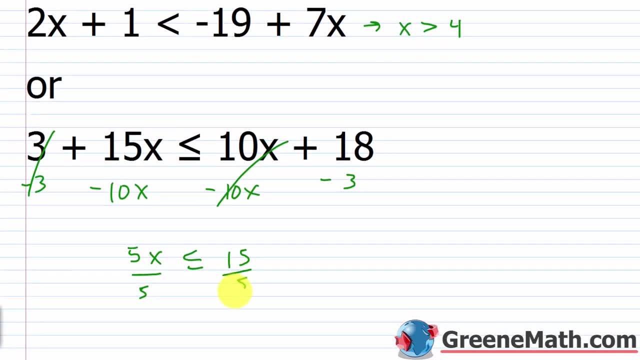 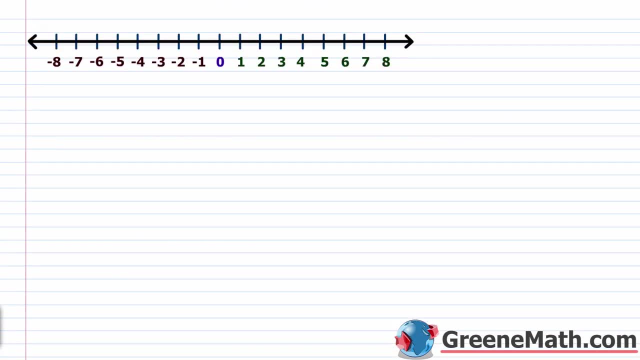 is 15. we divide each side by 5, we get that x is less than or equal to 3. this is: x is less than or equal to 3. alright, so we have that 2x plus 1 is less than negative 19 plus 7x. 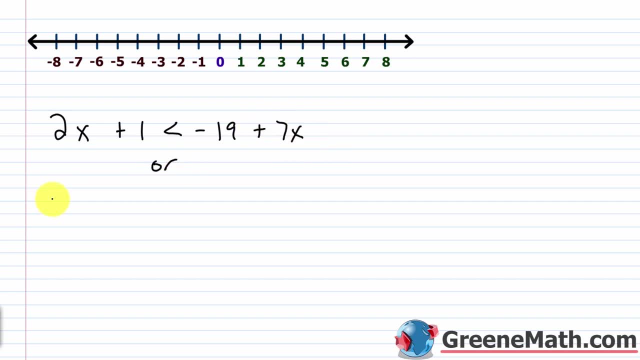 then or we have the other scenario: 3 plus 15x is less than or equal to 10x plus 18. so for this guy we found that the solution was: x is greater than 4, so in interval notation we would say that we would put a parenthesis at 4. 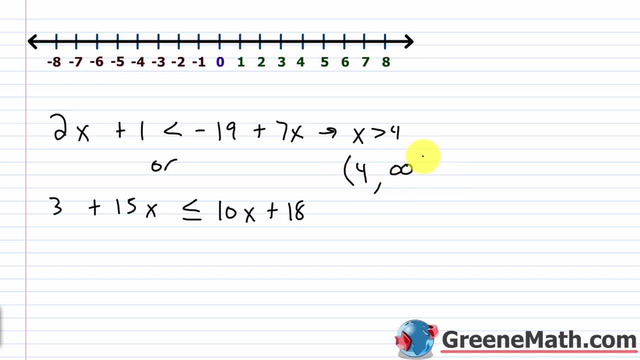 and then anything out, forever and ever and ever. so we put infinity here and then, graphically, at 4 I'd put a parenthesis facing to the right and I'd shade all of this now for this guy right here. we found that x was less than or equal. 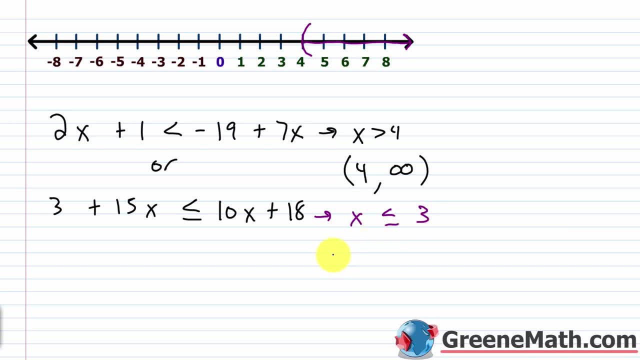 to 3. so in interval notation there's no smallest value. so we put negative infinity, put a parenthesis next to that and it's going up to and including 3. so we put a bracket next to 3. graphically I put a bracket at 3. 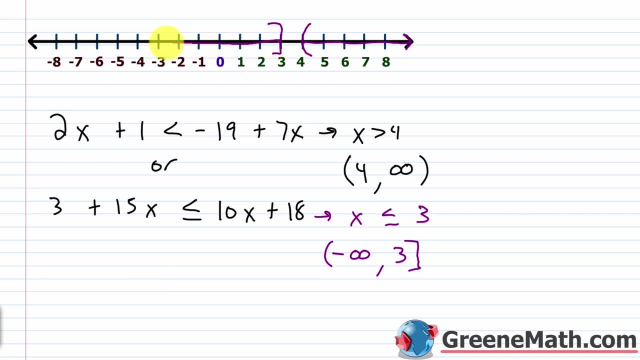 facing to the left, and then I shade everything to the left, and I'm going to shade this arrow now. you can see that there's no overlap between the two solutions. so if this wasn't an, or if this was an, and you would have no solution for the compound inequality. 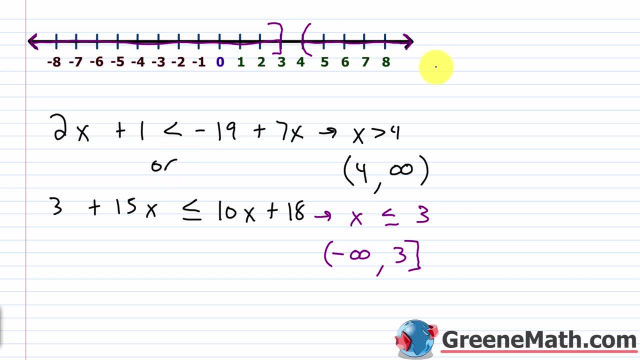 but because this is or and it can be a solution to either, to be a solution for the compound inequality, it's the union of the two solution sets. so, in other words, it is this guy right here. so it's negative infinity, up to and including 3. 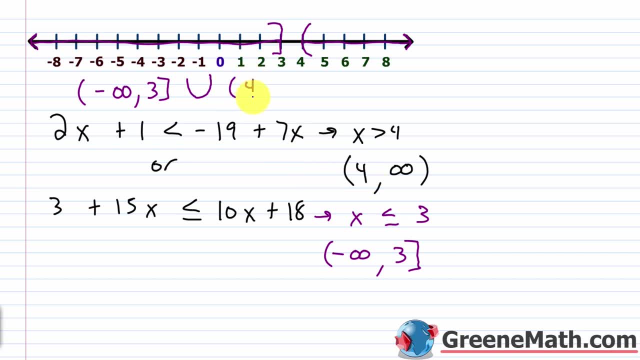 it's the union with this guy. we have 4. that's not included. we have the parenthesis there out to infinity. graphically, it's just this. I don't need to change anything. I've graphed each one, so I don't need to do anything else. 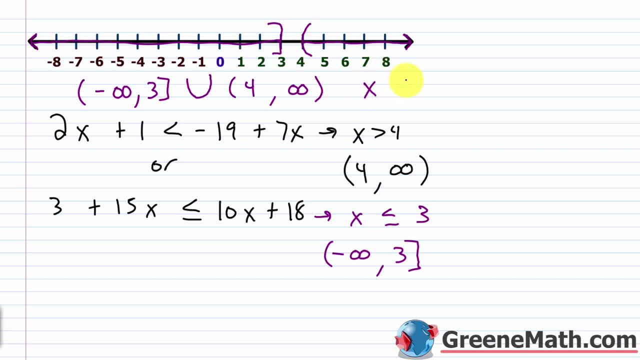 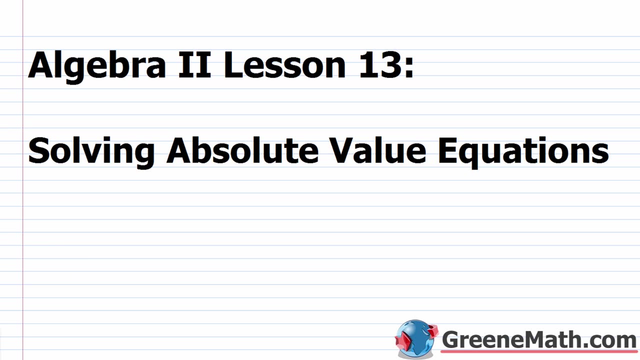 and then you could also write it as saying x is less than, or equal to 3, or x is greater than 4. each of these would show you the solution for that compound inequality. hello and welcome to algebra 2, lesson 13. in this video, we're going to learn about solving. 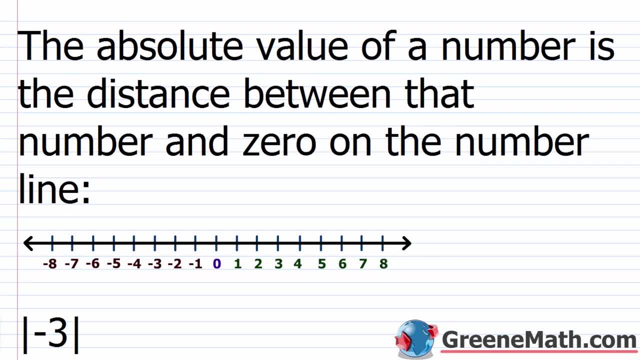 absolute value equations. so for most of you in an algebra 2 course this is a new topic. most algebra 1 courses do not go into this. it's considered a little bit advanced, but some of you might have seen it before. the main thing here is just to have a fundamental 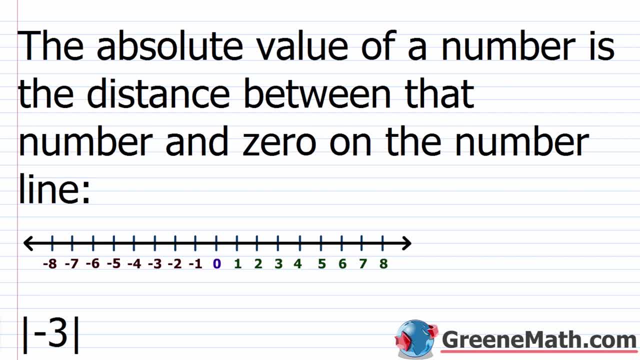 understanding of absolute value. everything else we're going to do is very, very easy, so I want to start with just a brief review. talk about things that we learned a long, long time ago and you might have forgotten. so the absolute value of a number is simply the distance. 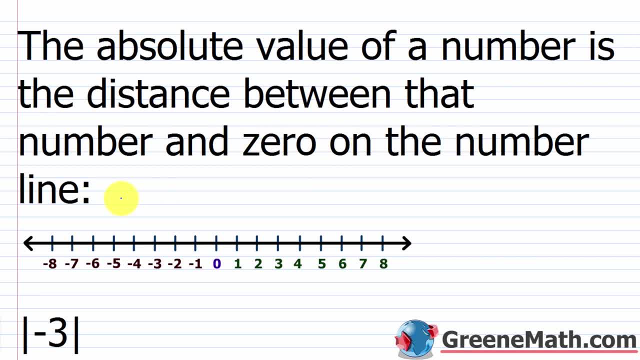 between that number and 0 on the number line. I want you to remember that absolute value is either 0 or it's a positive value. it's never going to be negative because, again, it represents a distance. it's kind of like if I get in a car and I want to drive somewhere. 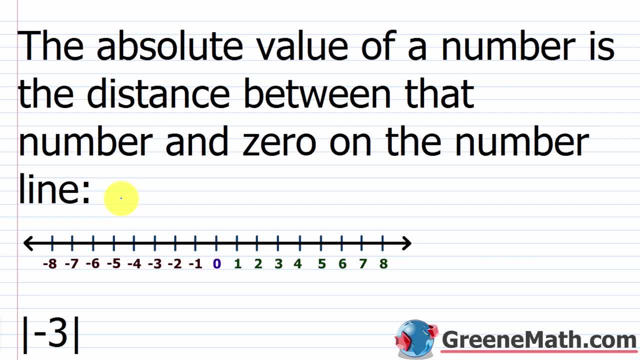 I can drive 0 miles or I can drive some positive amount, but I cannot go a negative amount. I don't want to hear the joke where you're going to get in your car and go backwards. that's not going to work. but I have some examples. 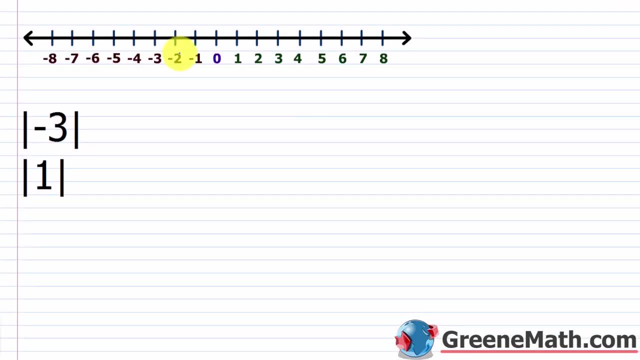 here just two brief examples. here's a number line and let's say we want the absolute value of negative 3 and again these bars here denote we want to take the absolute value of what's inside. so what is the absolute value of negative 3? well, I find negative 3 on the number. 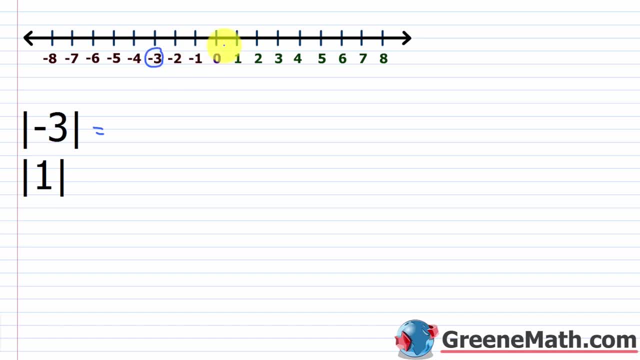 line that's here and I just travel to 0. how many units would I go? well, I would go 1, 2, 3 units and I'd end up at 0, and it doesn't matter what direction I go and it's how far I need to travel. so my absolute value. 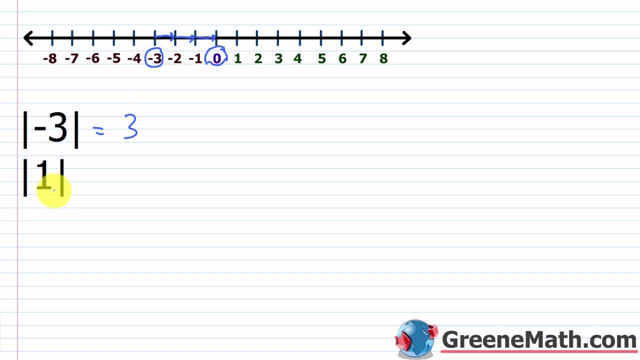 there would be 3 as another example, if I wanted the absolute value of 1. well, I'm coming from a different direction here, but I'm just traveling 1 unit to 0, so the absolute value of 1 is 1. basically, I know that all of you remember. 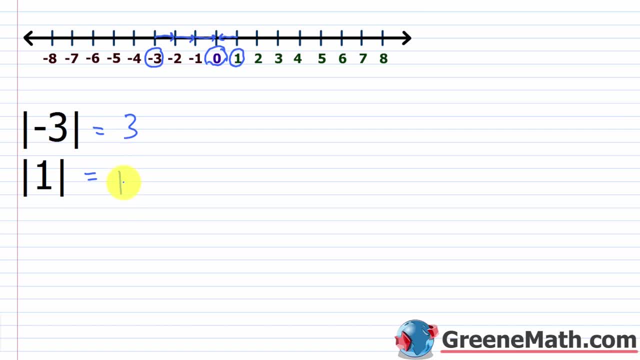 that the absolute value of a number, if it's positive, is just the number. the absolute value of a number if it's negative is just the opposite of it. right, just make it positive. so if I went through a few and said: what is the absolute value of? 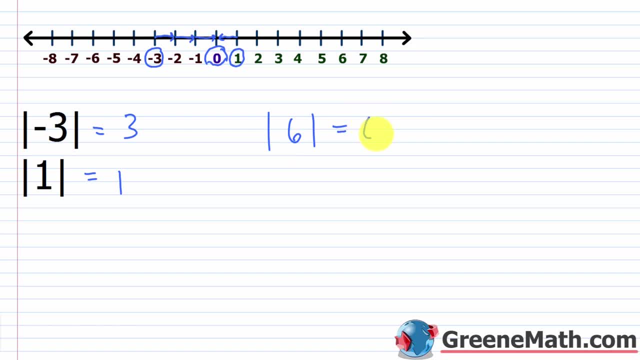 let's say 6. well, it's a positive number, so it's just the number, and I can kind of erase this and look at the number line and say, okay, well, the absolute value of 6. I can find that by just going from 6 to 0, and it's just what. 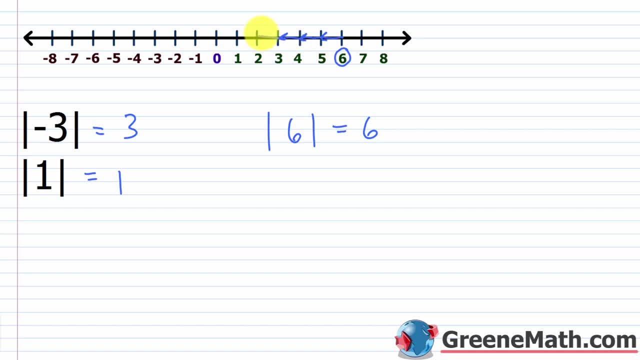 it's 1, 2, 3, 4, 5 and finally 6 units traveled to 0. okay, that's why the absolute value of 6 is 6, and the same thing would be true if I went from negative 6 to 0 from here. 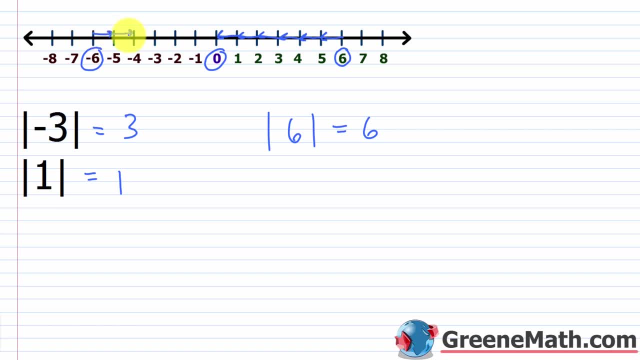 to 0 is also 6 units. it's 1, 2, 3, 4, 5 and finally 6. so the absolute value of negative 6, I would just make it positive- and it's 6. so that leads me to my next point here, and that point is that 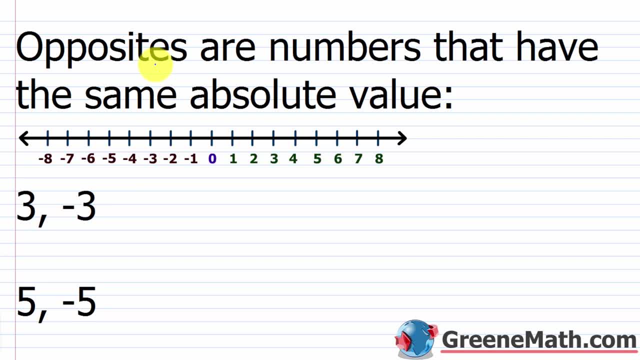 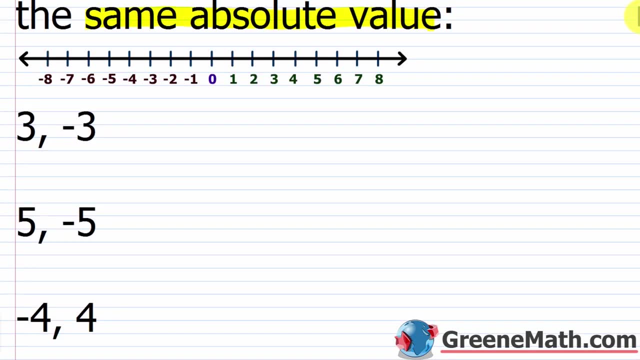 opposites, or we call them negatives or additive inverses, whatever you want to refer to them, as are numbers that have the same absolute value. okay, the same absolute value. very important. you understand that for this lesson. now I want to show you a couple of examples here and you can come up with. 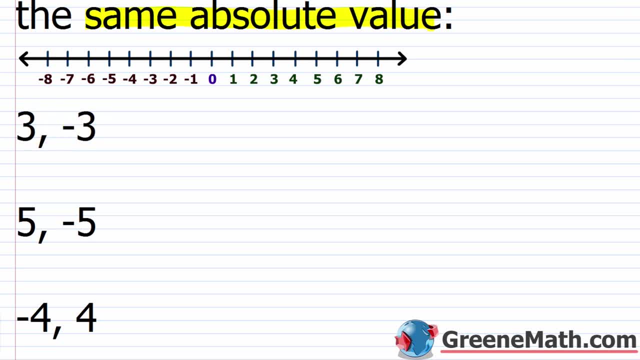 as many as you wanted to, but something like 3 and negative 3. if I take the absolute value of 3, it's equal to 3. if I take the absolute value of negative 3, it's equal to 3. so 3 and negative 3 are opposites and they have the same. 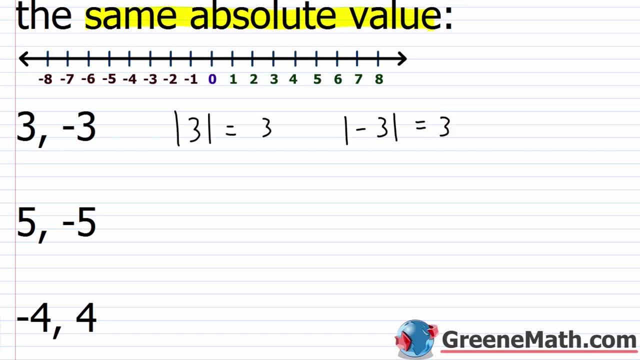 absolute value and again you can show that on the number line. you can go up here and say: okay, well, this is 3, this is negative 3 and each is 3 units away from 0. this is 1, 2, 3 units away from 0 and this is. 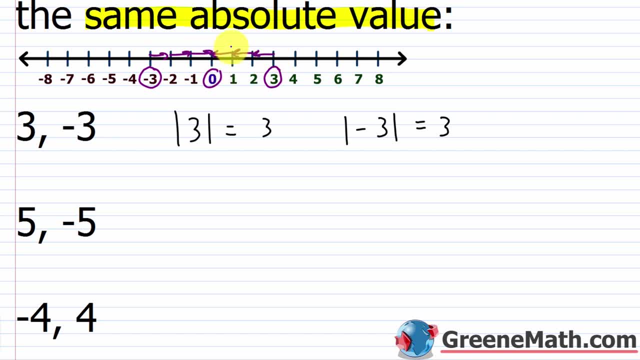 1, 2, 3 units away from 0 as well. and again, it doesn't matter which direction you're going in, you're just counting how far away you are from 0. it'd be kind of like if I was north and I traveled 500 miles to a. 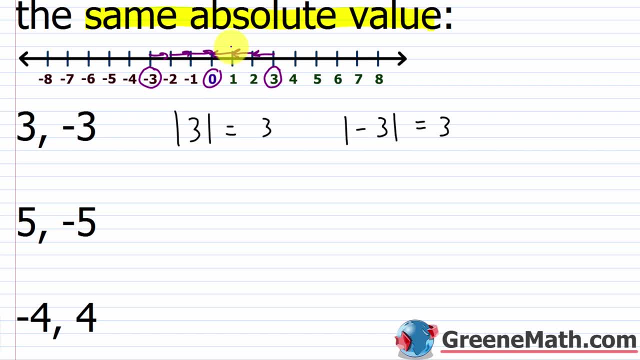 location. or if I was south and I traveled 500 miles to a location, it wouldn't matter where I came from, it's just a matter of it's 500 miles to get there. okay, so that's the concept of absolute value. so these I don't have to show graphically. I think we get it at this. 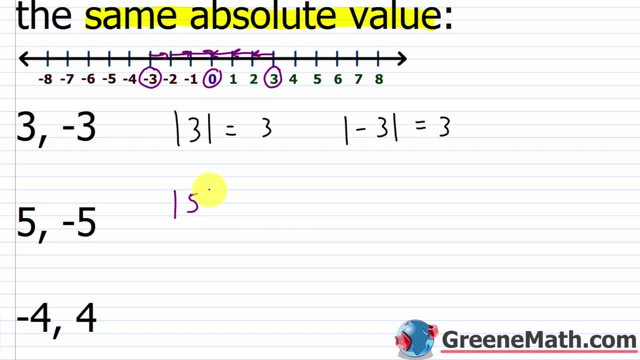 point. we know 5 and negative 5. if I take the absolute value of 5, I'd get 5. if I take the absolute value of negative 5, I would get 5 as well. negative 4 and 4 if I take the absolute value of negative. 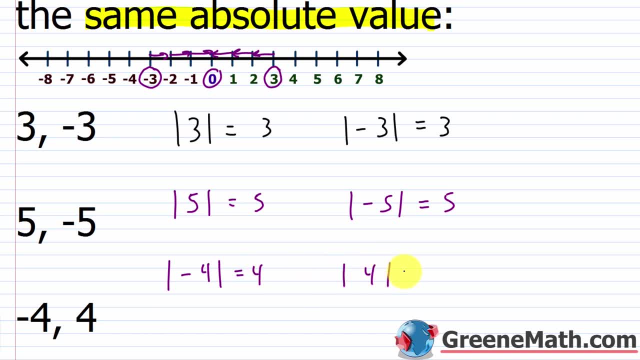 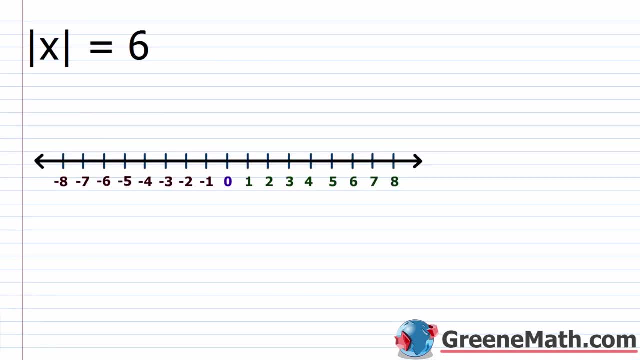 4, I get 4. if I take the absolute value of 4, I get 4. so anytime you have opposites, the absolute value is the same. now let me go to the first example that you're going to see in your textbook or that you're going to come across in class. 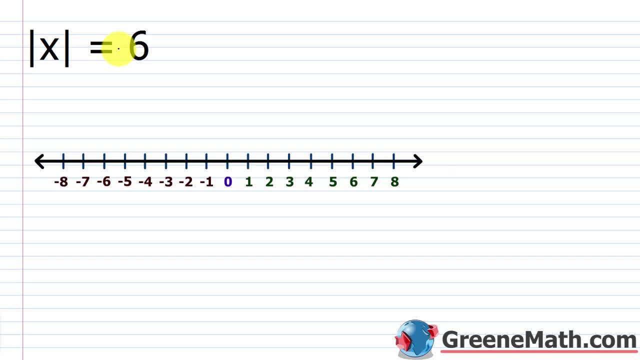 so you'll get something simple like this: the absolute value of x equals 6. so the question you have to ask yourself before you read anything, before you talk to anybody just thinking on your own: what could I replace x with to get a true statement? well, think about it. I want this to. 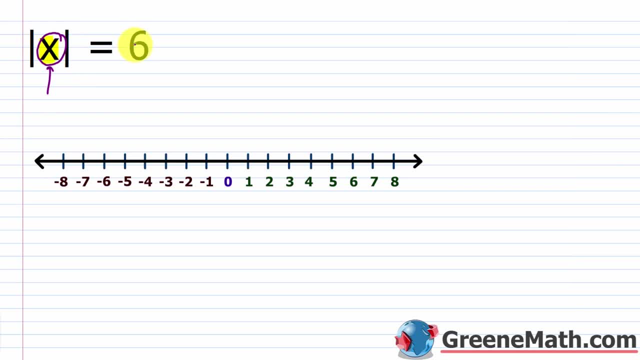 be some number that, when I take the absolute value of it, gives me 6 again. there are two numbers that have the same absolute value of 6. there's 6 and there's negative 6, because each is 1, 2, 3, 4, 5. 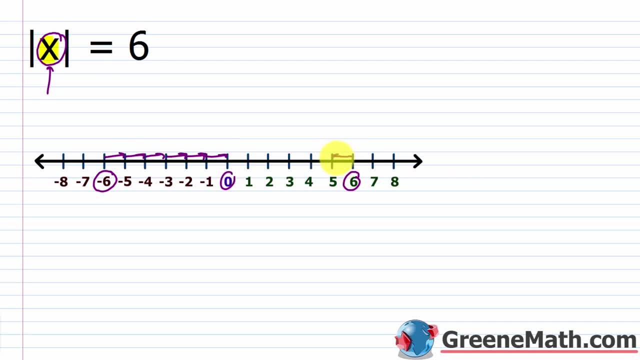 6 units away from 0 on that number line. this one the same thing: 1, 2, 3, 4, 5, 6 units away from 0 on the number line. so in this particular case, x could be equal to what it could be. 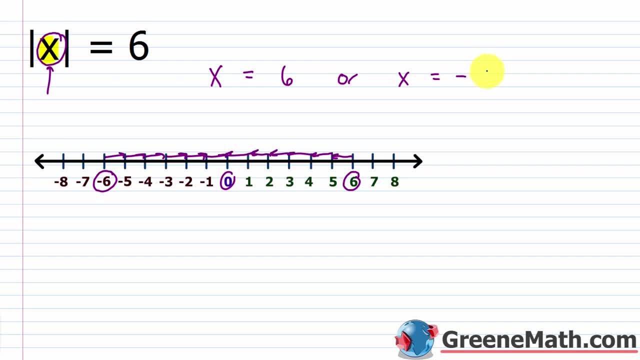 6 or x could be also negative 6. if I plug in a 6 there, I take the absolute value, I get 6. if I plug in a negative 6, there I take the absolute value, I also get 6. as another example, let's say I had the absolute value of x. 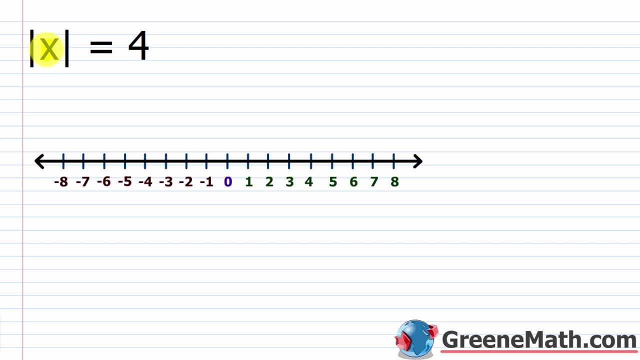 is equal to 4. again, what could x be here? well, there's two possibilities: it could be 4, or it could be negative 4, because each would have an absolute value of 4, right? so it could be x could be 4 or x could be negative 4. 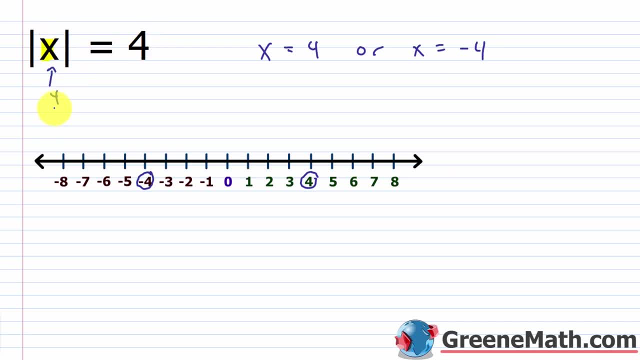 again. plug in a 4: here absolute value of 4 is 4. plug in a negative 4 here: absolute value of negative 4 is 4 as well. and again you can just show yourself this on the number line. this is 1, 2, 3, 4 units. 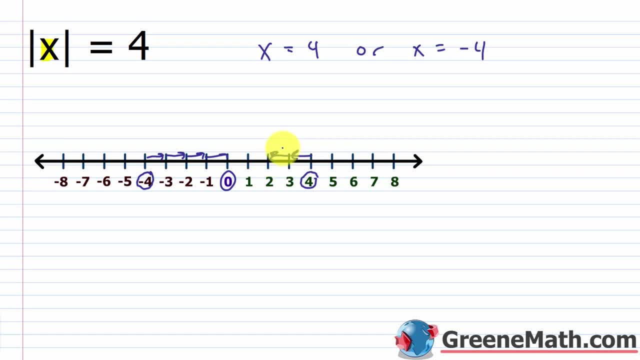 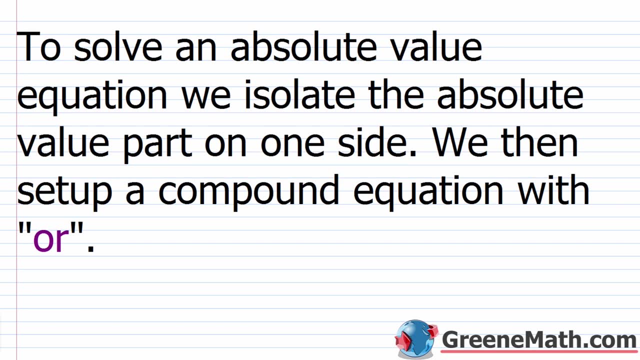 away from 0, and this is 1, 2, 3, 4 units away from 0 as well. so obviously that's the easiest scenario you're going to come across, but you use the same concept when you get into the harder ones to solve an absolute value equation. 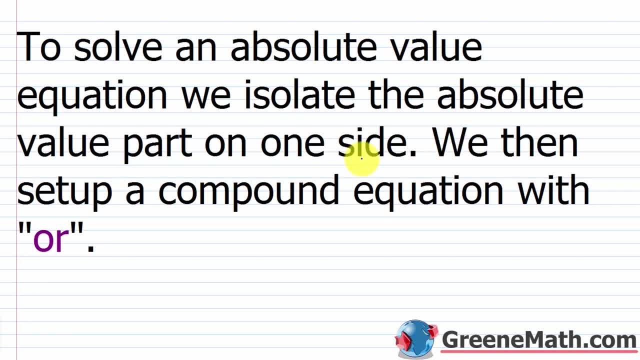 we isolate the absolute value part on one side. we then set up a compound equation with: or, okay, remember, or is telling you that either solution is going to work. so let's look at an example. so we have the absolute value of 6n plus 10. 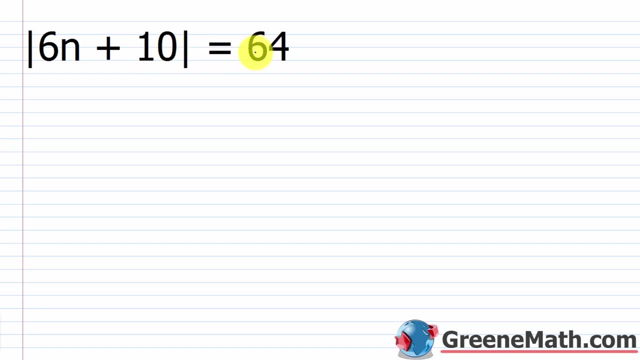 is equal to 64. so what we need to do? again, if this is isolated for us, we can say that 6n plus 10- this is inside of absolute value bars- can be equal to positive 64. let me put a plus out there for emphasis. 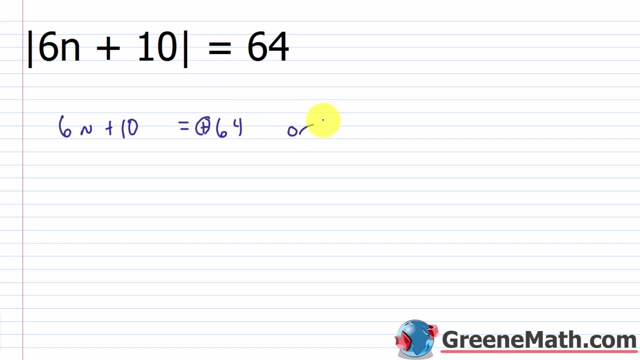 or it could also be equal to the negative of 64. so 6n plus 10 could be equal to negative 64. you might say, well that I don't know. that doesn't make much sense. we go back to the last example where we had. 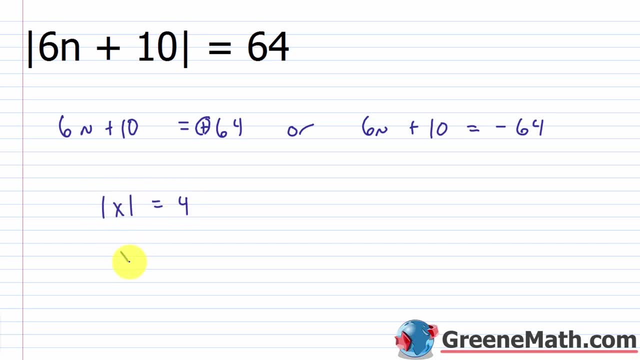 the absolute value of x was equal to 4. well, this is. x could be equal to 4, or x could be equal to negative 4. it's the same principle here, it's just a little bit more advanced. and remember, I could plug in a 4 here. take the absolute value, I get 4. 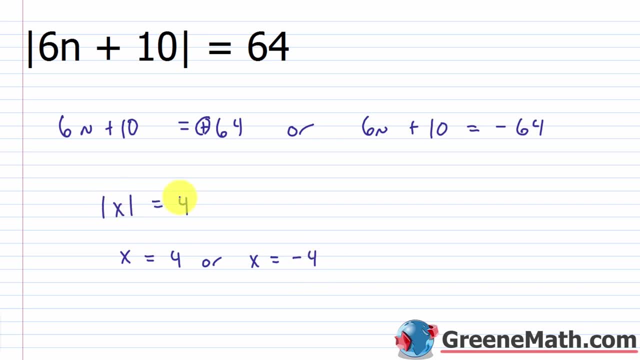 I could plug in a negative 4 here. take the absolute value, I get 4. both of these would work. what I am saying here is I've got to solve for n and I want a value for n that when I plug it in here, I'm going to multiply it by 6. 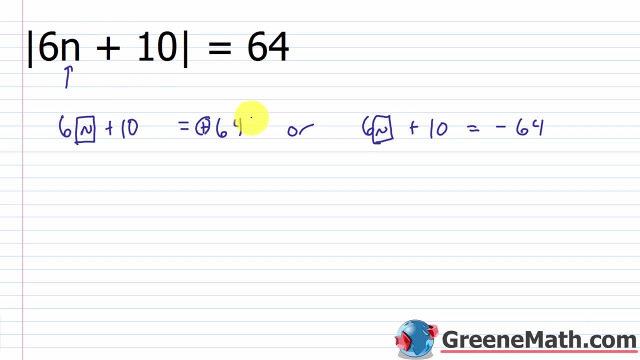 I'm going to add 10. the result, I'm saying, could be 64 positive 64, or it could be negative 64. it makes no difference, because the absolute value operation will make it positive, right, if it's positive, it stays positive. if it's negative, 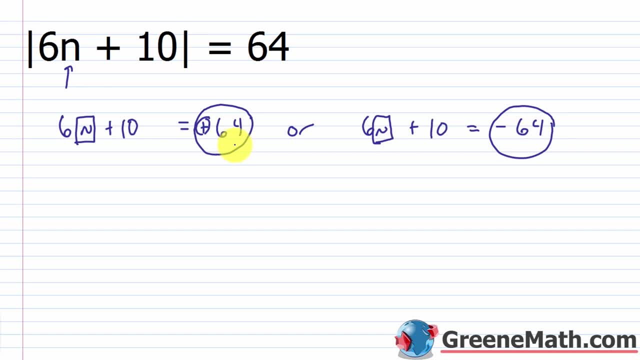 it's going to become positive. I don't care if I get 64 or negative 64, because either way I'm going to get a solution to the equation. so let's go ahead and solve each one of these and we're going to plug both of them in, and I'm going to prove to you that. 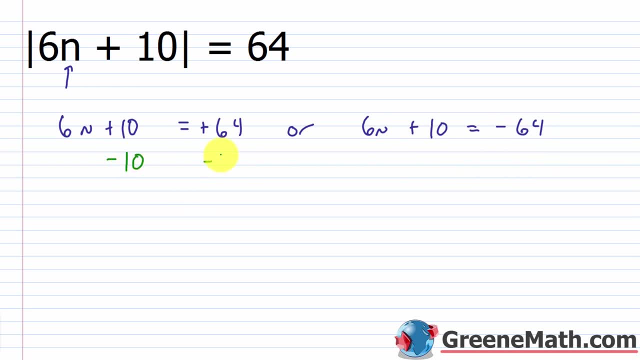 works either way. so for this one I'm going to start out by subtracting 10 away from each side, and this will cancel. I'll have 6n is equal to 64 minus 10 is 54. I will divide both sides by 6, so that n is. 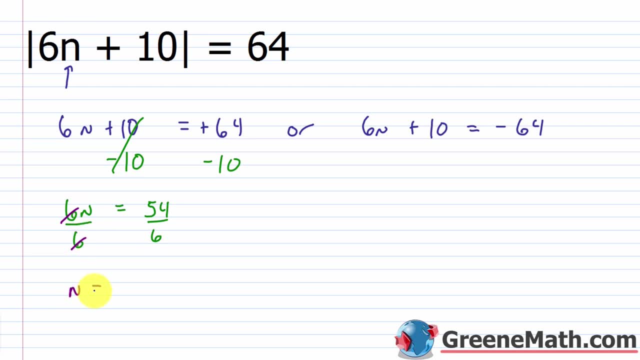 by itself. so this will cancel with this and I'll have: n is equal to 54 divided by 6, is not? so that's one solution. then we have our or so we have another scenario. so we're going to subtract 10 away from each side, over here as well. 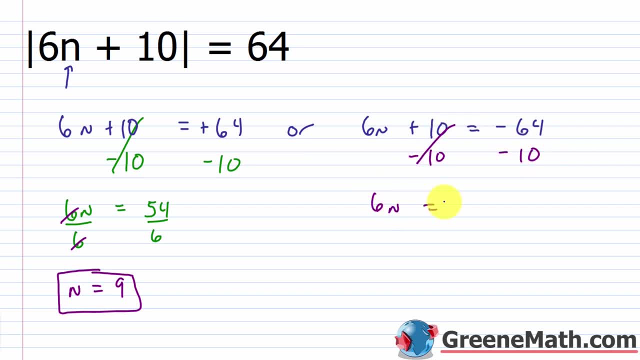 that will cancel, I'll have: 6n is equal to negative 64 minus 10 is negative 74. if I divide both sides by 6 here, this will cancel with this and I'll have n is equal to, so negative 74 over 6. I can reduce. 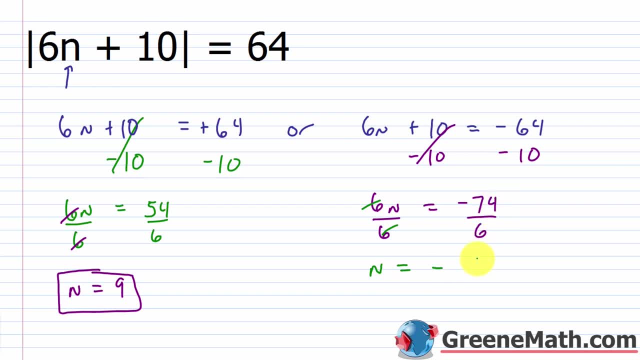 this- I know it's going to be negative- 74 is divisible by 2, 74 divided by 2 is 37, and 6 divided by 2 is 3. so there's my other solution. so I'm going to put or here, and let me erase this part. 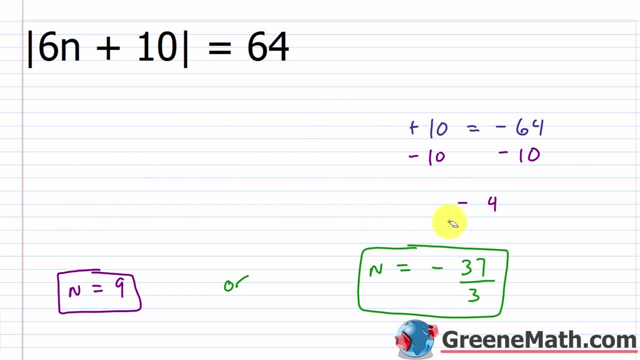 and I'm going to show you that they each work. I'm also going to write this in solution set notation. again, we've got to get more used to doing that. so in solution set notation, remember, I create some set brackets and inside those brackets I'm going to put my solutions. 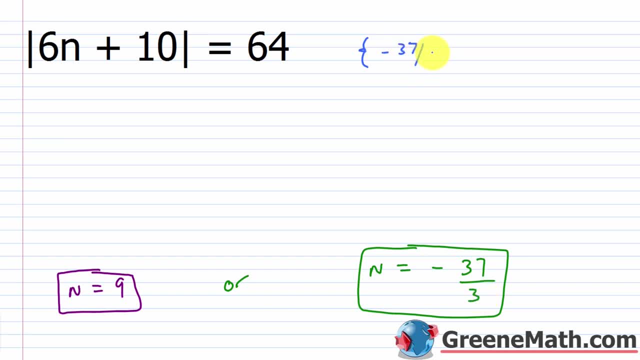 as the elements. so I have negative 37 thirds comma. the other element is 9. that's my other solution. so I want to check these two and I want to show you what happens when we plug them in again. n is equal to 9 or n is equal. 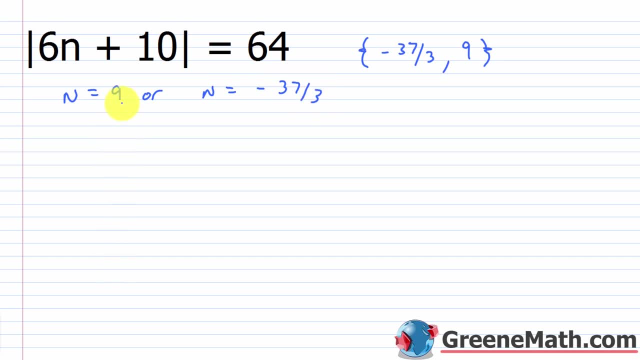 to negative 37 thirds. so the first one, n, equals 9. so what happens when I plug in a 9 for n? so you have 6 times 9 plus 10, and then we take the absolute value of this and it should equal 64. 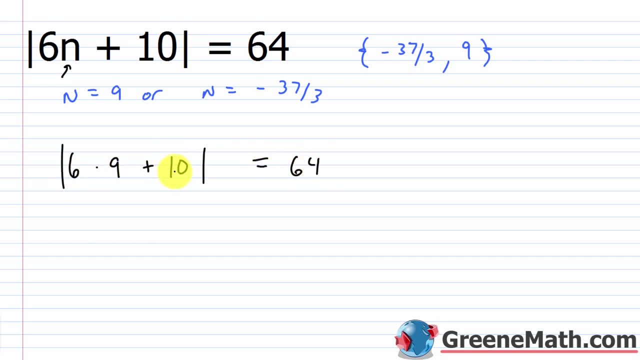 well, 6 times 9 is 54, 54 plus 10 is 64. so you get the absolute value of positive 64, which of course is going to equal 64. so the left and the right side here are going to be equal. so that's our first scenario. 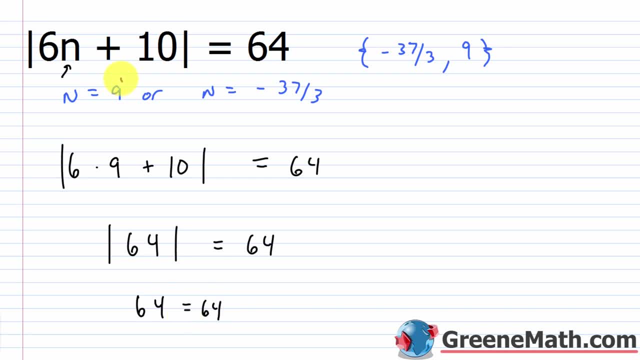 that's kind of the easy one to understand. the second scenario is the one where it kind of takes a little bit of thought into absolute value to understand. so for this one let me kind of back this up a little bit, because I'm dealing with a fraction here. 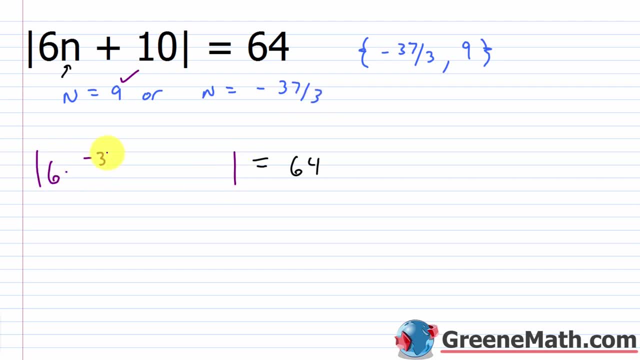 so it will be a little messier. so I have 6 times negative, 37 over 3. that's what I'm plugging in for n, then plus 10, and I want the absolute value of this guy, and it should equal 64. so I know that. 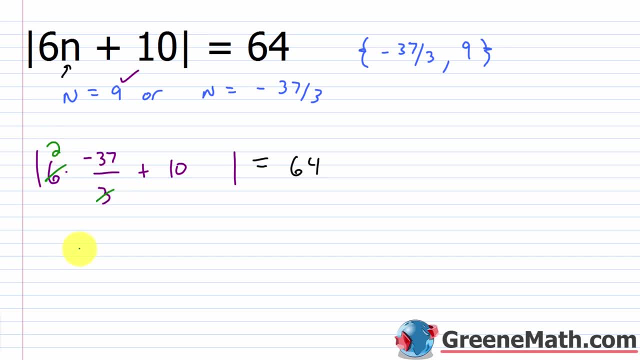 this will cancel with this and give me a 2, 2 times negative 37, as we know, is negative 74, so this would be the absolute value of negative 74 plus 10, and this should equal 64. negative 74 plus 10 is negative 64, so this would be the absolute. 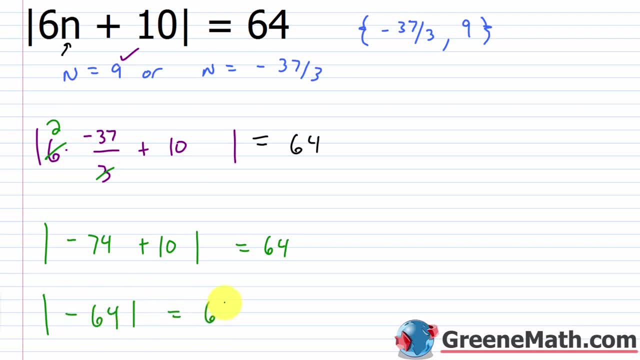 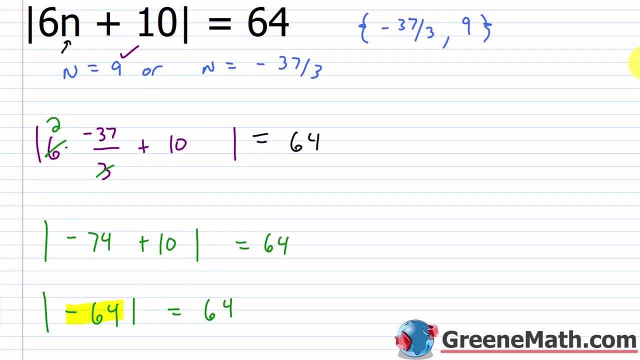 value of negative 64 is equal to 64. now, again, when I take the absolute value of negative 64, it's going to make it positive. so the two sides are going to be equal because of the absolute value operation. so that's why we end up with two solutions here. 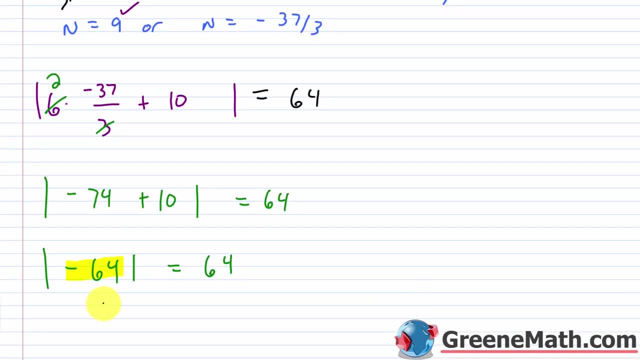 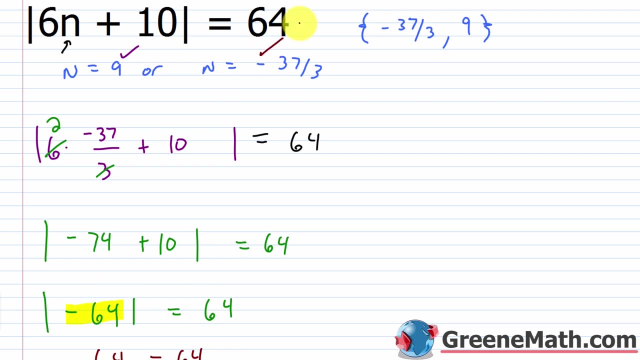 so this- I'm going to scroll down a little bit- turns out to be: 64 equals 64, and so this is good to go. so what we can say here is that this solution is correct as well, and again, it's an important insight to understand why these two solutions work. 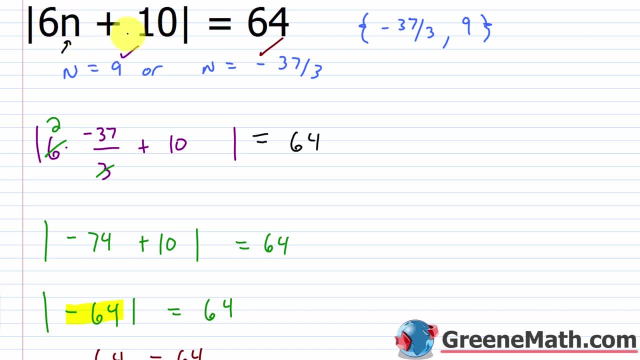 again, when I plugged in a 9 here, I got positive. 64 took the absolute value, I got 64 equals 64. when I plugged in a negative 37 over 3 in for n, I got negative. 64 took the absolute value of that, I got positive. 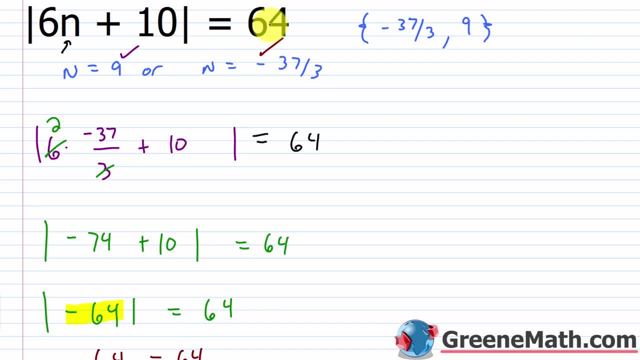 64. so it might be still a little bit confusing, but we're going to work a lot of examples here, so let's go to the next one. so for the next one, it's a similar setup. we have the absolute value of 10x plus 10. 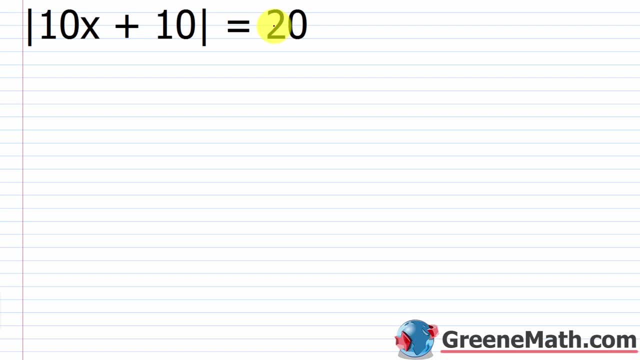 this is equal to 20. so again, what I'm saying is that what's inside the absolute value operation, which is 10x plus 10? well, that could be equal to 20, but also I'm going to put, or this could also be equal to negative 20. 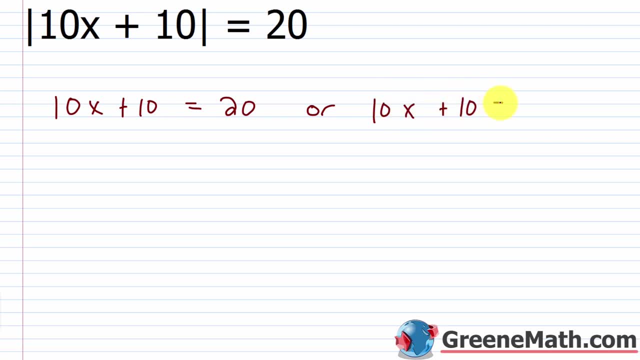 so 10x plus 10 could be equal to negative 20. you set up these two scenarios, you set up a compound equation with or again, because if I find something for x that, when I plug it in, makes this whole thing equal to 20, I'm good. 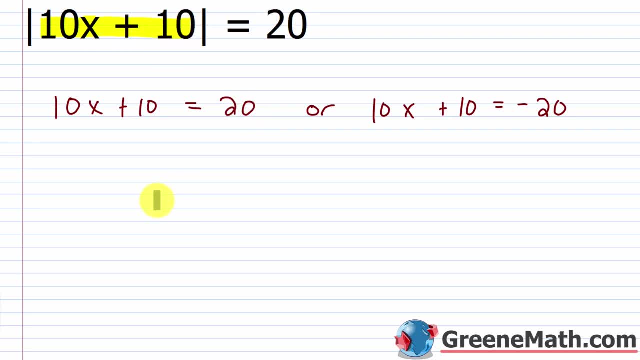 right, the absolute value of 20 would be 20. additionally, if I find something that I plug in for x and it makes this whole thing equal to negative 20, I'm also good, because the absolute value operation will make that negative 20 positive 20. so again you've. 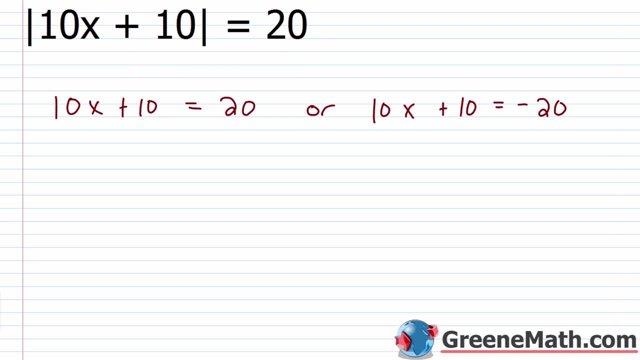 got to think about those two different scenarios. let's go ahead and check this out. so we would subtract 10 away from each side of the equation here. that would cancel. I'd have: 10x is equal to 20 minus 10 is 10. divide both sides by 10. 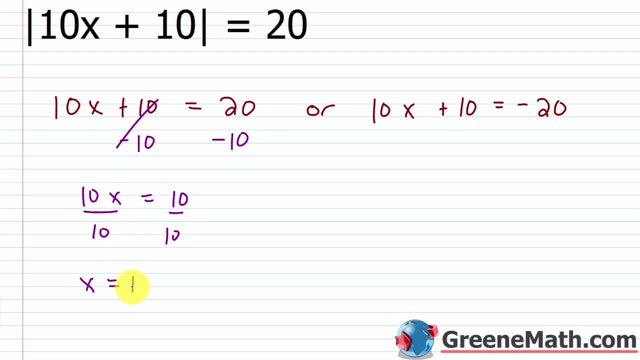 and we would get x is equal to 1. over here, let's subtract 10 away from each side of the equation. that cancels, I'll have 10x is equal to negative 30. divide both sides by 10, we'll get x is equal. 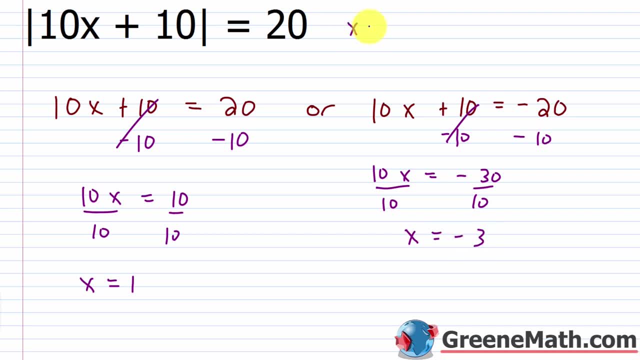 to negative 3. so what we find here is that x equals 1 or x equals negative 3. in solution set notation I would say negative 3 and 1 are my elements. right, they're my two solutions. let me erase this real quick. I'm not going to check all of these, but 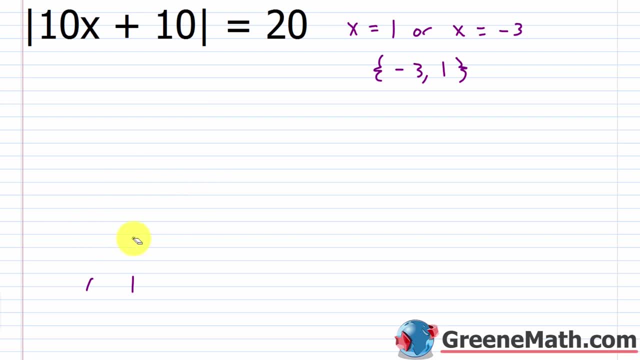 I will check a few just to kind of pound the point home that this value inside could end up being 20 or negative 20 and you're going to end up with the same value on each side once you take the absolute value. so if I start out by plugging in a 1 for x, 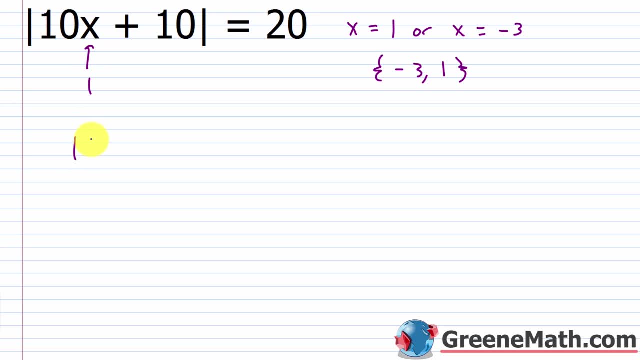 the obvious scenario: 10 times 1 is 10. so I'd have 10 plus 10 and I'd take the absolute value of that and that should be 20 and of course, 10 plus 10 is 20. so the absolute value of 20. 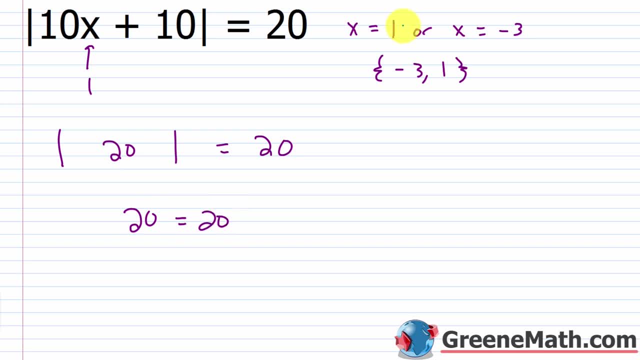 is 20, you get. 20 equals 20, so of course we are good to go there. the other one again, that's the one that confuses people and that's the one that people just don't think about. so if I plug in a negative 3 there, I would have the absolute. 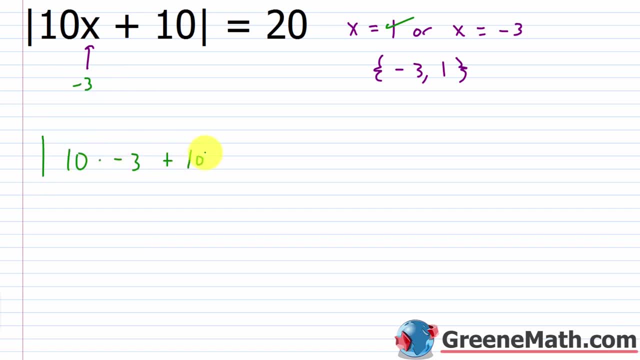 value of 10 times negative 3 plus 10. this should equal 20. 10 times negative 3 is negative 30. so I would have the absolute value of negative 30 plus 10, which is negative 20, and this should equal 20. 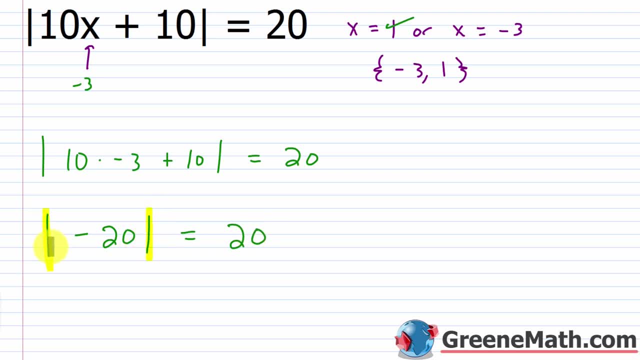 again, the absolute value operation here is what allows us to have a negative 20. when I take the absolute value of negative 20, I get positive 20. ok, so this becomes 20 and it equals 20. so 20 equals 20. that's true. 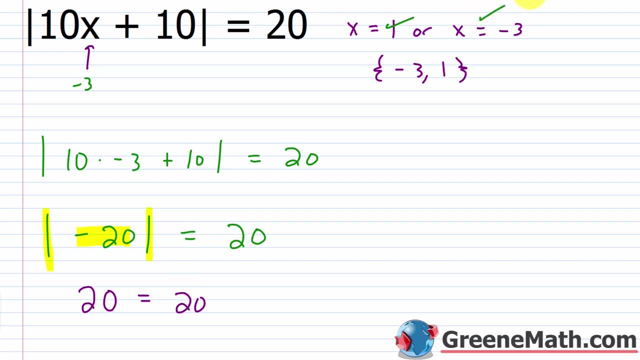 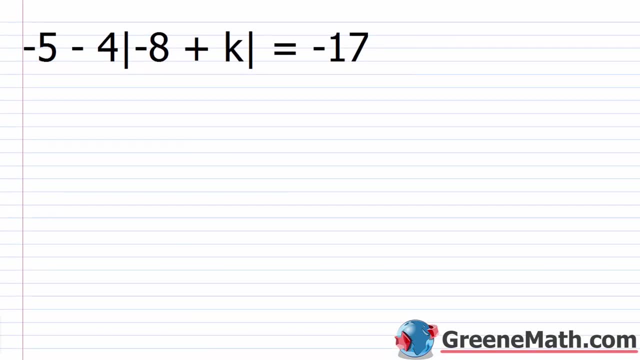 so this works out as a solution as well. so here, x can be 1 or, equally valid, x could be negative, 3- two solutions for this equation, alright. so now that we've gotten through the easier ones, let's look at a tougher one now. what do I do in this scenario? 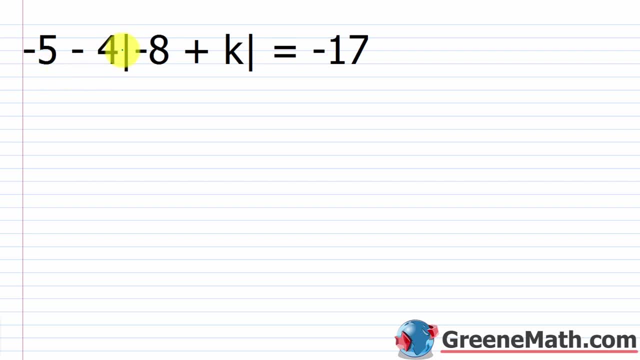 I have negative 5 minus 4, and this is multiplication because it's hanging out outside. so times the absolute value of negative 8 plus k is equal to negative 17. well, what we want to do is we want to isolate the absolute value operation. so we want to. 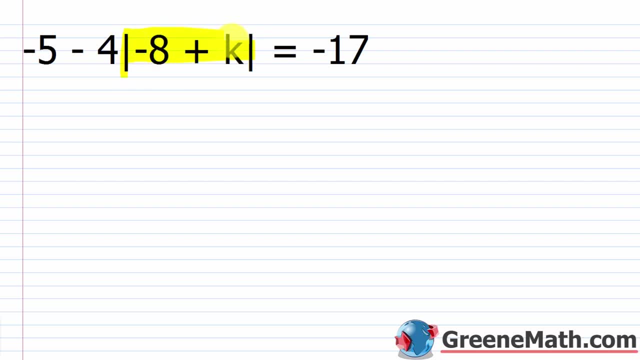 get this by itself, and we can do that because we happen to be very good at algebra at this point. so the first thing I'm going to do is I'm going to add negative 5 to each side of the equation, so this would cancel what I'm left with. on the left, I'd have negative 4. 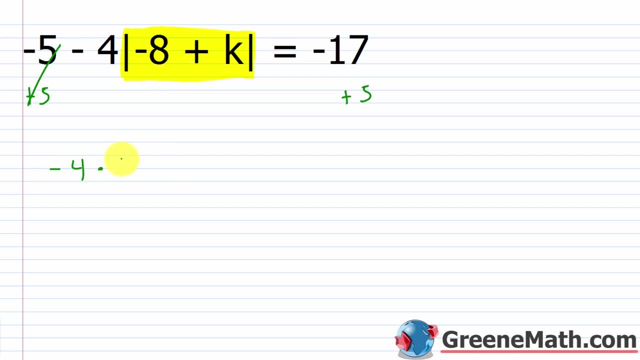 times. I'm going to put a multiplication symbol there. so it's obvious. the absolute value of negative 8 plus k, and this is equal to negative 17 plus 5, which is negative 12. now again, this is multiplication. I want this thing by itself. so if I have something multiplying something, 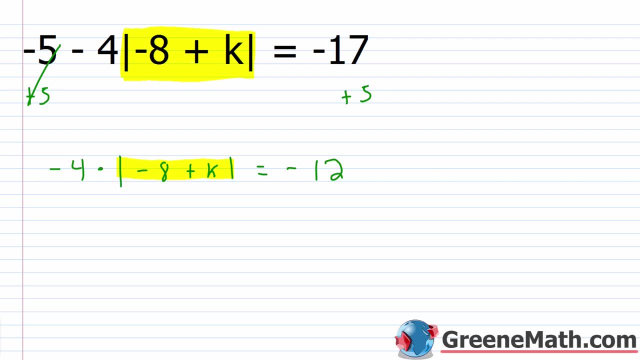 else and I want to isolate it. I'm going to use division, just like if I had 6x equals 30. I want to isolate this. I divide both sides by 6. right simple, it's the same thing. if I want to isolate this, I divide both sides by. 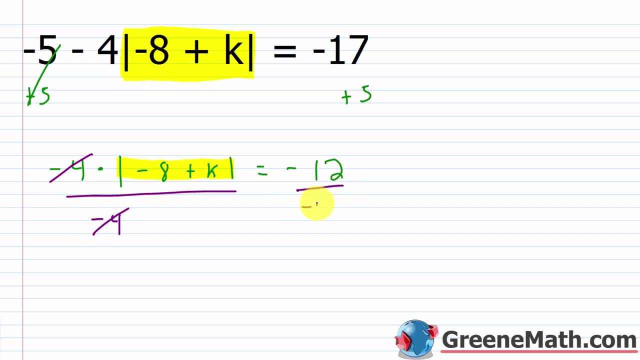 negative 4, because that's what I want to go away. so this is left: the absolute value of negative 8 plus k, and then, on the right side, negative 12 divided by negative 4 is simply 3. so now we have it in a format that we 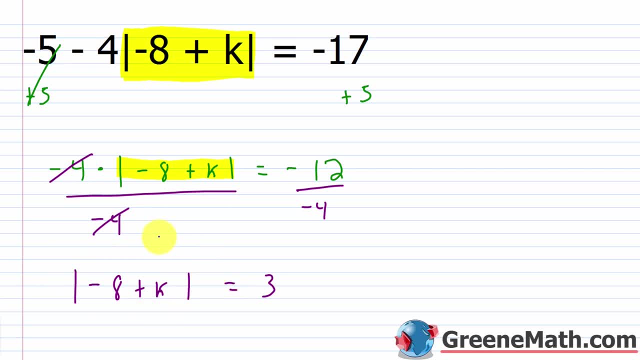 saw in the last two examples. it's all that you need to do: just get the absolute value operation isolated on one side, you want a number on the other and again you set up your compound equation. so this guy inside the absolute value bars can be equal to: 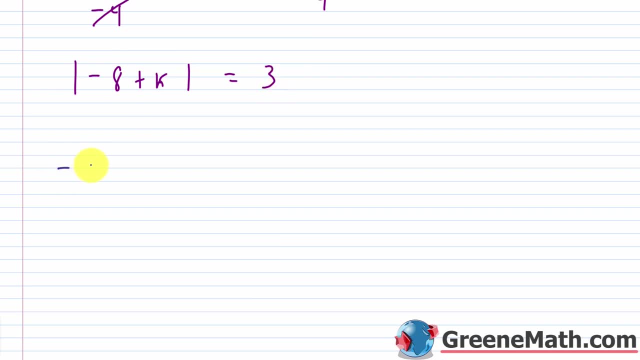 this or the opposite of that. so it is negative. 8 plus k is equal to 3 or negative. 8 plus k again could be equal to negative 3. if this was 3, it's good. if this was negative, 3, the absolute value operation makes it. 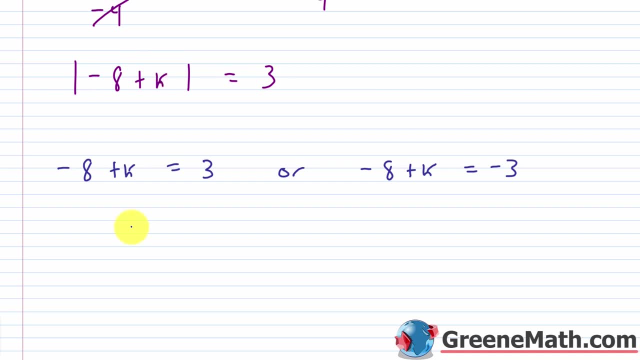 good as well. okay, so to solve these very, very simple equation: add 8 to each side. over here, you're going to get that k is equal to 11, and over here, add 8 to each side and you're going to get that k is equal. 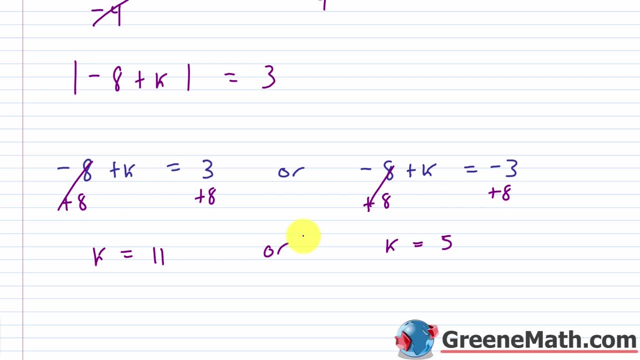 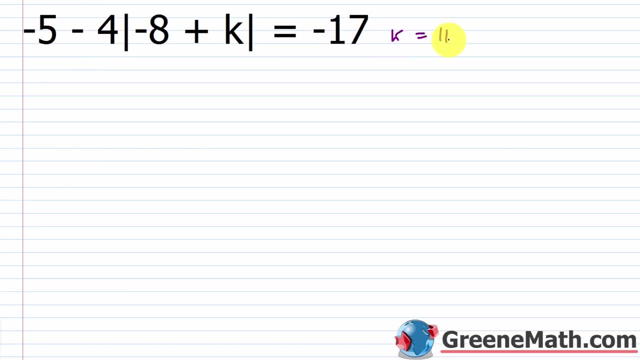 to 5. so I've got my solution of k equals 11 and then my other solution of k equals 5. so let's erase everything. we're going to check that again. we have that k equals 11 or k equals 5, and again using 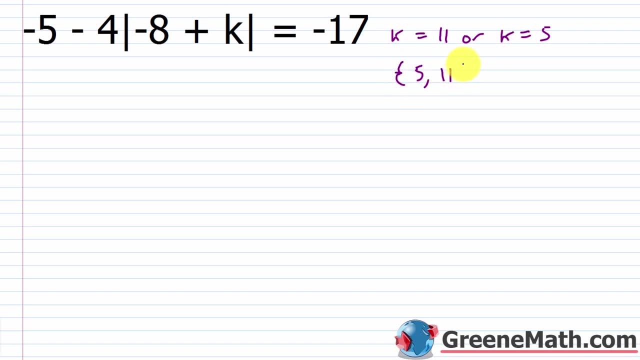 the solution set, notation 5, comma 11. that's going to be my two elements. so let's start by just plugging in a 5. so I plug in a 5 there, so I'd have negative 5 minus 4. let me make that negative a little better. 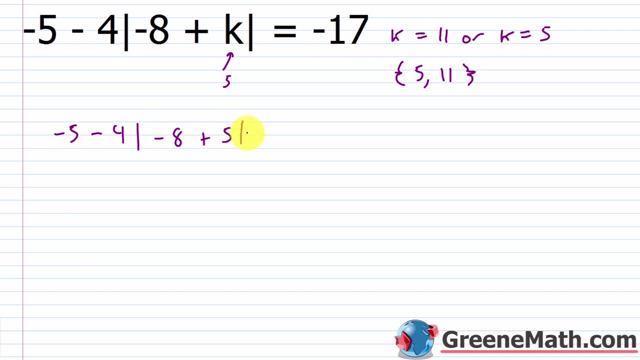 and then this times the absolute value of negative 8 plus 5, and this equals negative 17. so negative 8 plus 5 is going to give me a value of negative 3. so this would be negative 3. remember this is multiplication, so down here I'd have negative 5. 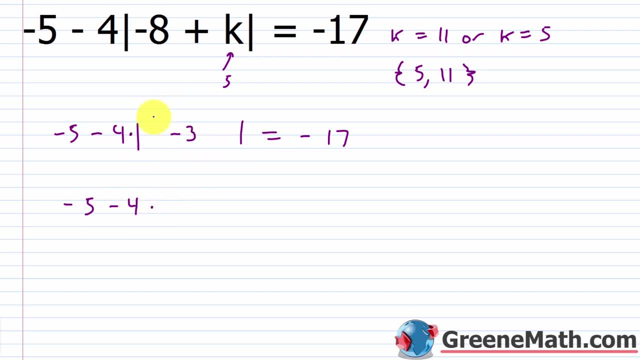 minus 4 times again. the absolute value operation makes this positive 3. this should equal negative 17. so I do multiplication before I do anything else. you can think about this as plus negative. to make it easy, negative 4 times 3 is negative 12, so you'd have negative. 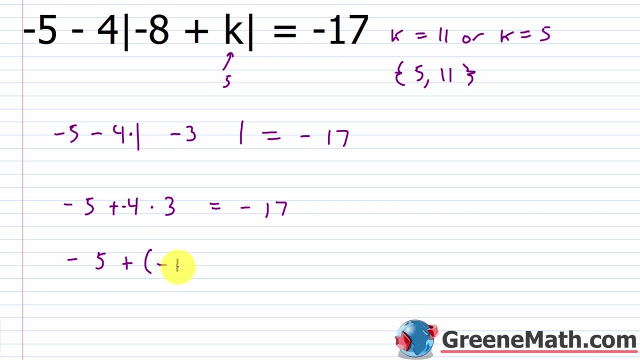 5 plus again this is negative 12 and this should equal negative 17, and it does. negative 5 plus negative 12 is negative 17. so our solution of k equals 5 is correct. alright, for the other one, we want to try k equals 11, so you'd. 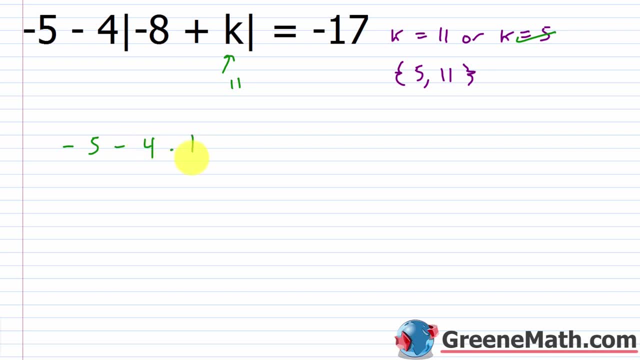 have negative 5 minus 4. again, times the absolute value of negative 8 plus 11, this equals negative 17. so negative 8 plus 11 is 3, so let me replace this with 3, and again the absolute value of 3 is 3, so I'd have negative 5. 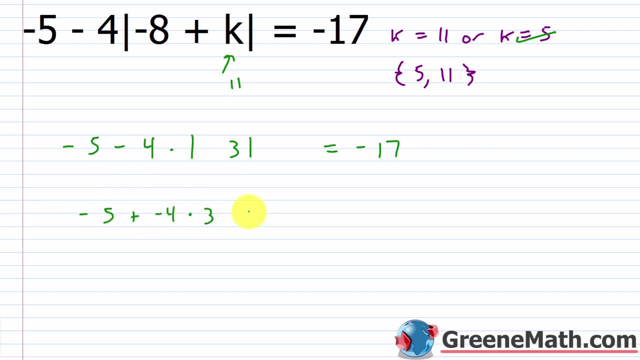 I'm going to write this as plus negative. 4 times 3 equals negative 17. it's the same thing, because the absolute value operation, whether it's 3 or negative 3, puts out a positive 3, so either way I got the same thing. 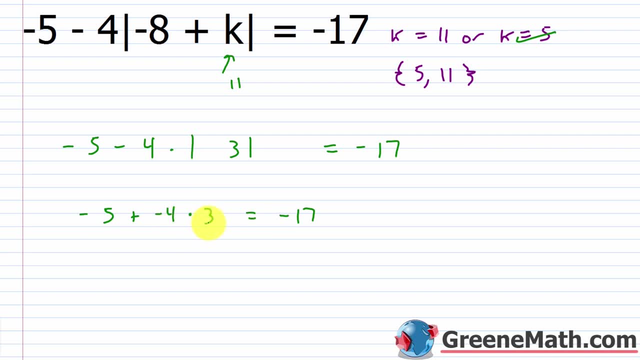 here. the rest of it's the same. negative 4 times 3 is negative 12. you get negative 5 plus negative 12 equals negative 17. this is negative 17 equals negative 17, so this checks out as well. so k here can be 11. 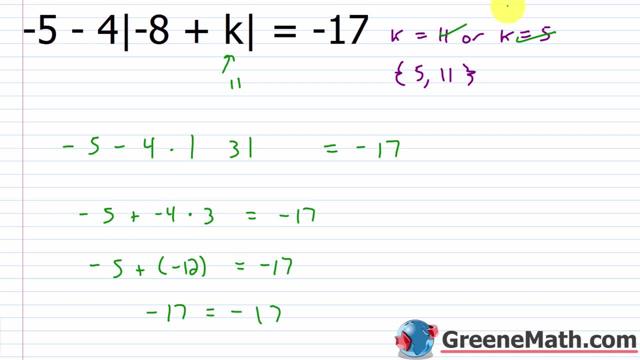 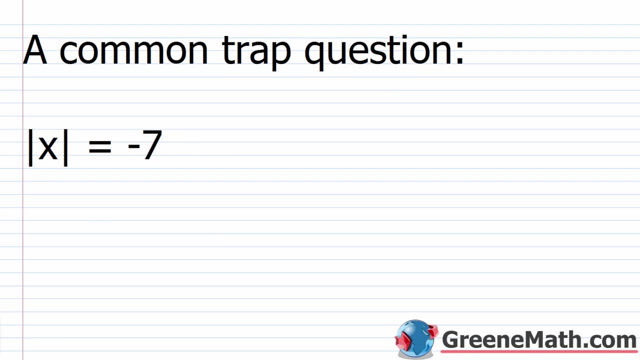 or equally valid k here can also be equal to 5. alright, so the next 3 problems I'm going to give you are going to be trap questions that you're going to come across your teacher or your textbook. whoever you get information from your tutor, maybe just this video. 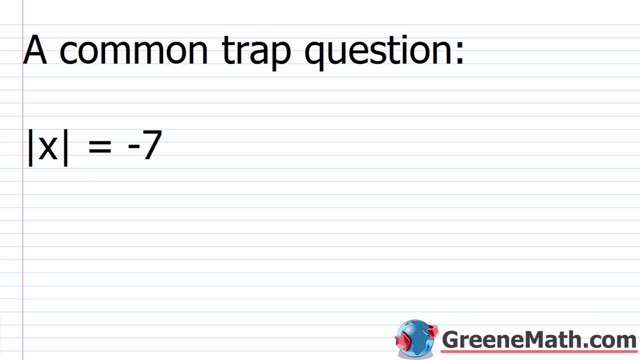 somebody's going to give you a problem that's going to look something like what you're going to see in the next 3 problems. so a common trap question would be something like this: the absolute value of x is equal to negative 7. again, why is that a trap question? go back. 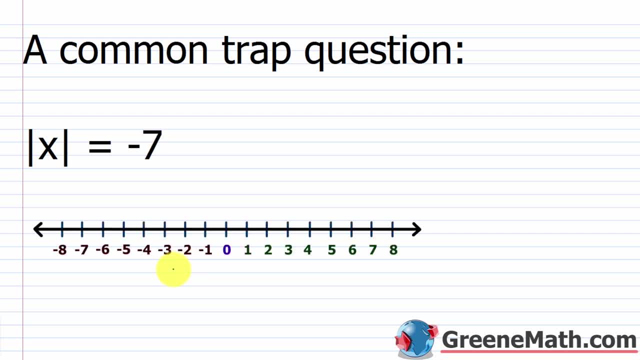 to a number line and I'll bring one to the screen there. tell me what number you have that has a distance from 0 of negative 7. it doesn't exist. you might say, oh well, 7. no, it doesn't work that way. 7 has a distance of. 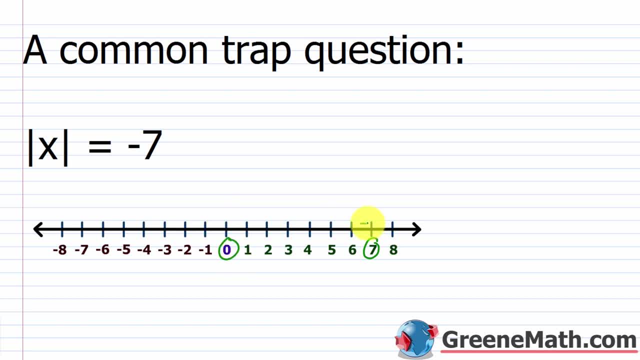 7 units away from 0. alright, if I counted, it'd be 1, 2, 3, 4, 5, 6, 7. the answer here is there is no such x because, as I told you, the very first part of this video, absolute value, is a distance. a distance is either: 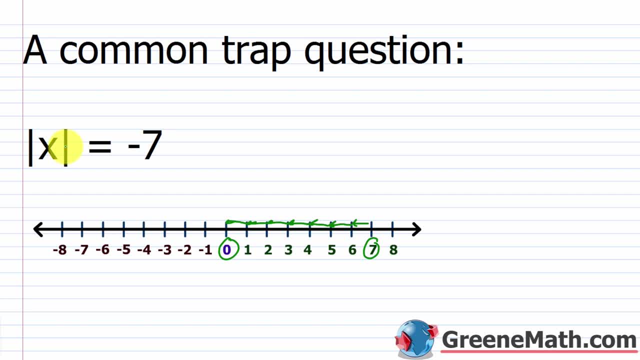 0, or it's positive. I get in my car, I want to go somewhere. I either start the car and it doesn't work and I don't go anywhere and I go: damn I'm not going anywhere today, or I go some positive amount, I do not go negative. 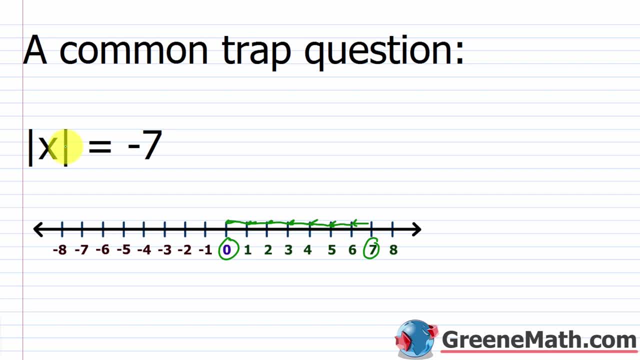 again, not with the joke about backing up. that doesn't work. so for this particular type of problem, there is no solution. there is no solution. okay, you can also put the symbol or the null or empty set right, because the solution set contains no elements and you just want to remember that. whatever, 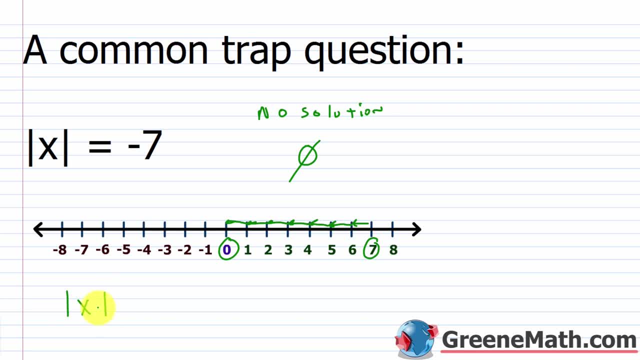 is inside the absolute value bar. you can just say the absolute value of x, for example. this is always greater than or equal to 0. it can be 0 or positive, it cannot be negative. so this is not going to work alright. so let's look at an example. 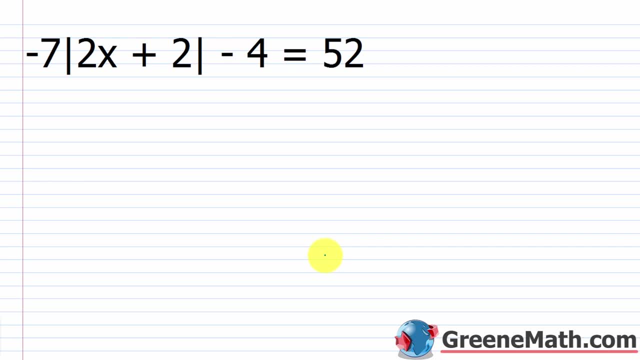 so you see something like this: it looks nice and normal. you're like: okay, I'm ready to get my solution. so you have negative 7 times the absolute value of 2x plus 2 minus 4 equals 52. okay, so I'm going to start. 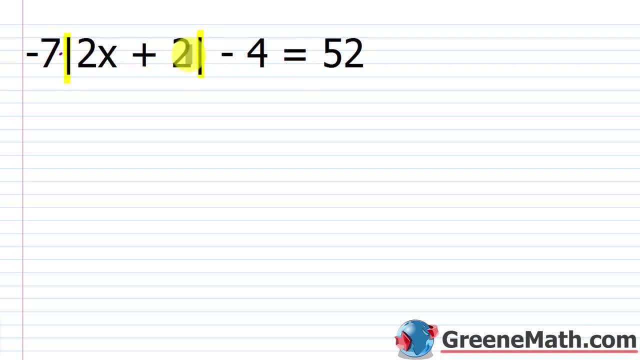 by trying to what? isolate this? I want to isolate this, so I'm going to add 4 to each side. that's going to give me negative 7 times the absolute value of 2x plus 2. this would cancel. it would be equal to 52 plus 4. 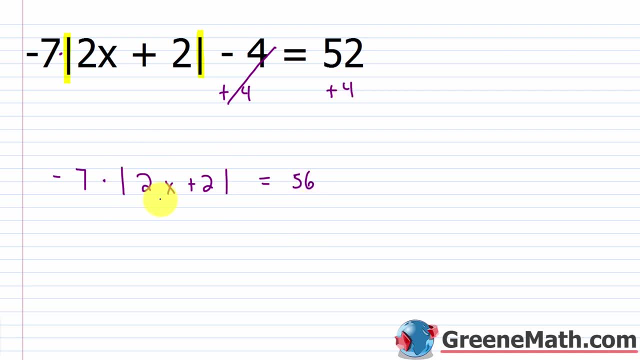 is 56. now, if I want to isolate this again, if I'm isolating this and this is being multiplied by that, well, I want to divide both sides by this so I can get rid of it. so this would cancel with this and over here, 56 divided. 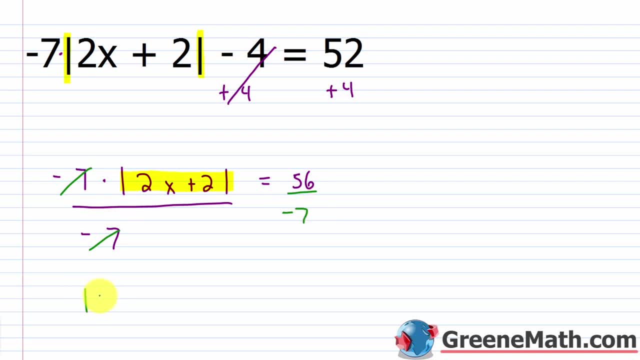 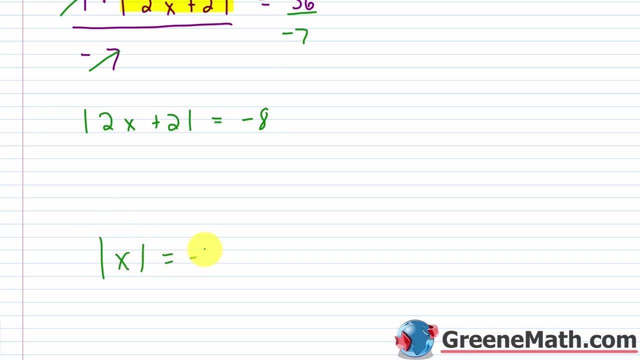 by negative 7 is negative 8. so I now have: the absolute value of 2x plus 2 is equal to negative 8. is there a problem? yes, there is. I know this is a little bit more complex than me just saying the absolute value of x is equal to negative 7. 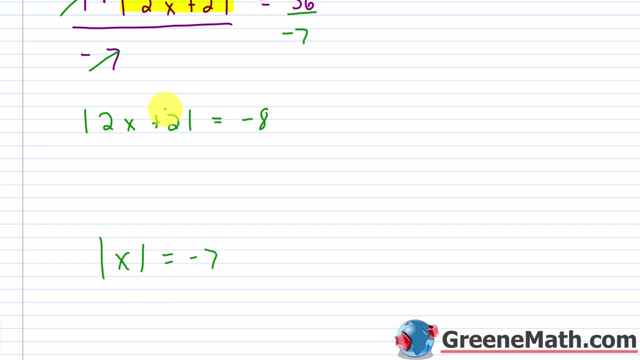 that's obvious. this one right here. somebody might start thinking: yeah, I can make that work. I can go: 2x plus 2 equals negative 8, or 2x plus 2 equals 8. I see students do this all the time. it's not going to work. 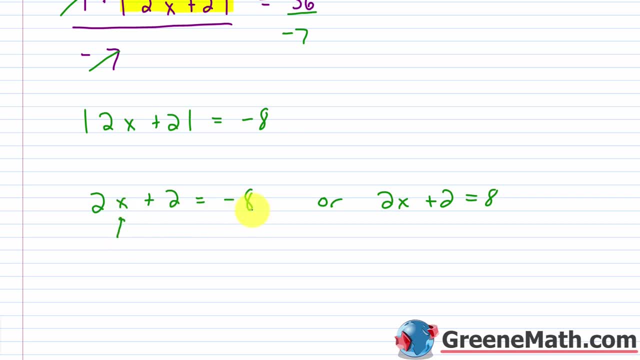 stop and think about it. I can find an x here that's going to give me a value of negative 8 when I evaluate. so let's go ahead and do that. I'm going to show you what happens. let's subtract 2 away from each side of the equation. 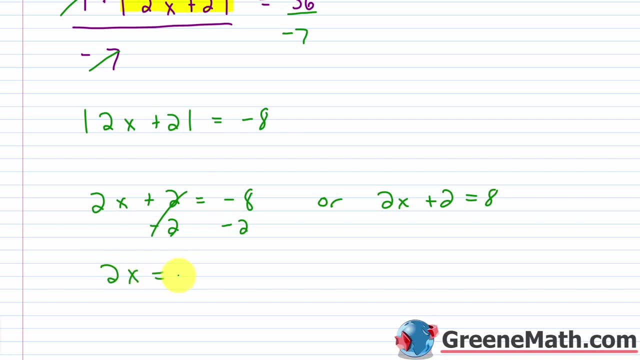 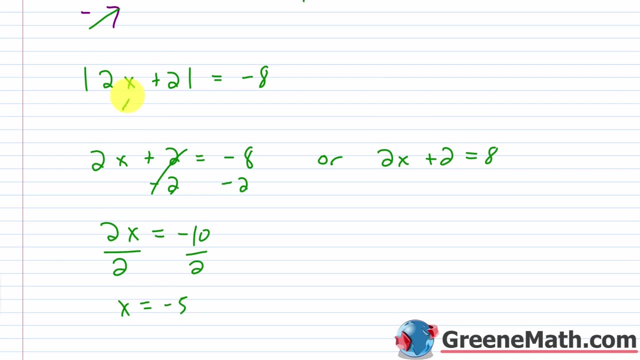 and that will cancel. you'll have: 2x is equal to negative 10. divide both sides by 2, you get x equals negative 5. ok, so let's say I plug in a negative 5 here. what's going to happen? let me just erase this. 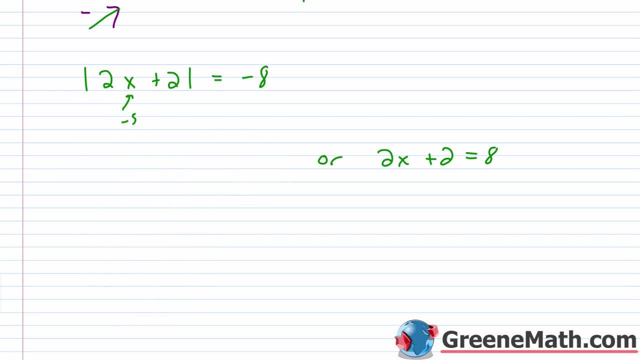 so we have a little room to work. we don't even need it anymore. so 2 times negative 5 is negative 10. so I have the absolute value of negative 10 plus 2 is equal to negative 8. now finish this up: negative 10 plus. 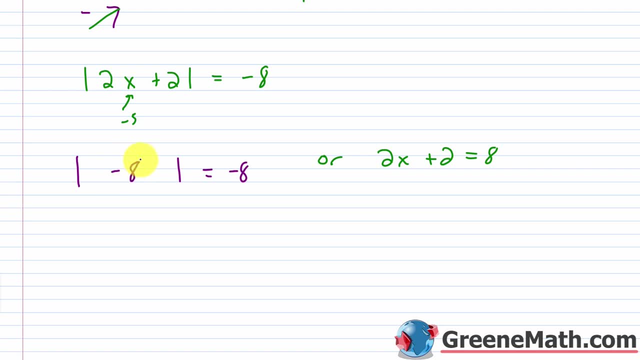 2 is negative 8 and you might say, oh, I nailed it. now I got negative 8 on this side. negative 8 on this side. hold on, it's inside of the equation. now I have the absolute value operation, so it's not going to work. 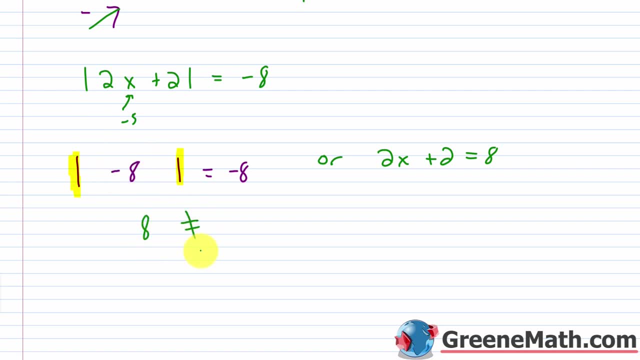 once I take the absolute value of this, it's positive 8. positive 8 does not equal negative 8, so this doesn't work. you can't do it that way. ok, if you isolate your absolute value operation and it ends up being equal to a negative. 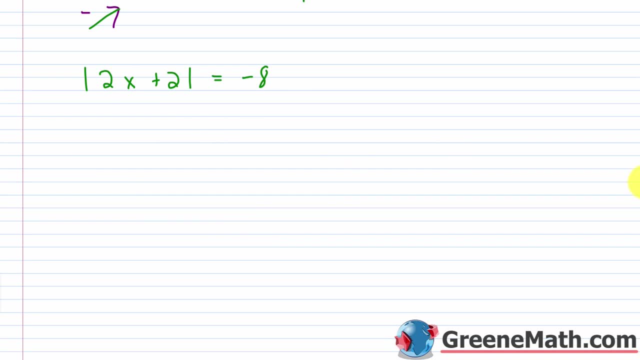 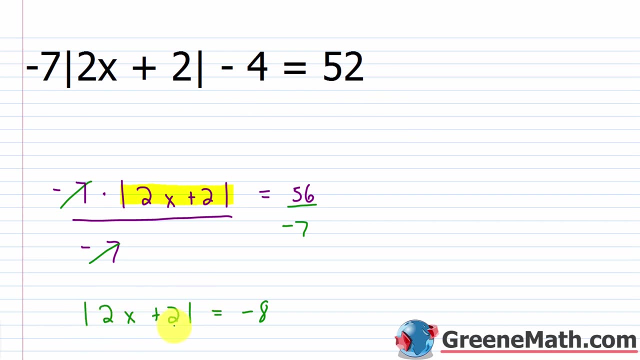 stop, there is no solution. ok, so when we come across a scenario like this and we go through all the work and we isolate it and we say, ok, the absolute value of 2x plus 2 is equal to negative 8, we stop. we say nope, they're not going to get me on this. 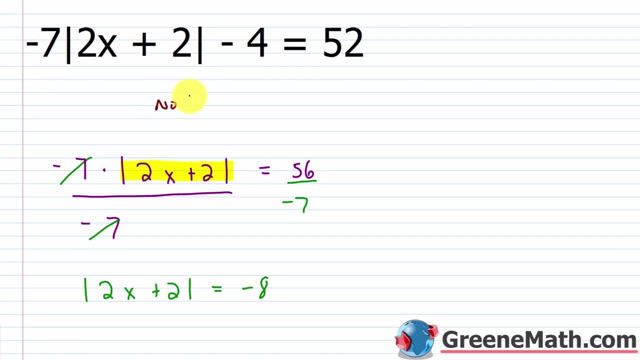 trap question and there's no solution. ok, put the symbol for the null or empty set, because again, no matter what you plug in for x there, once you take the absolute value of it, it's going to be 0 or positive. it will never, ever, ever be negative. so you can't possibly get a solution. 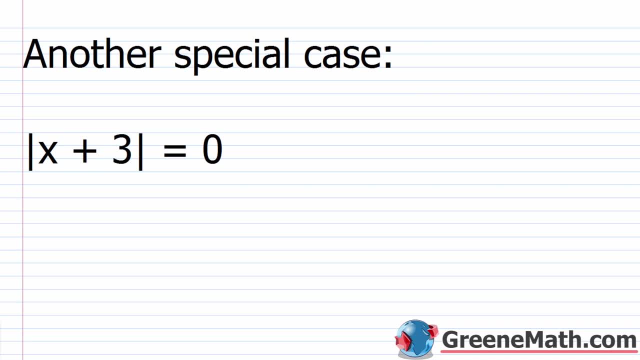 alright. so another special case is when you've isolated your absolute value operation and it's equal to 0. so here I have: the absolute value of x plus 3 equals 0. well, in this case you can get a solution, but there's only one possibility. 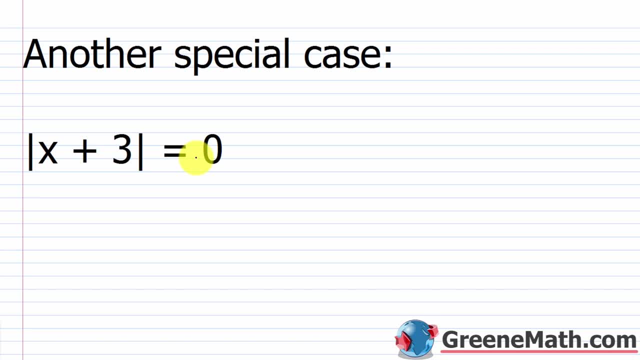 because 0 is its own opposite. right it's. it's absolute value is 0. it's 0 units away from itself by definition. if I look at a number line, just for reference, here's 0. how many units is it away from itself? 0. if I get on google. 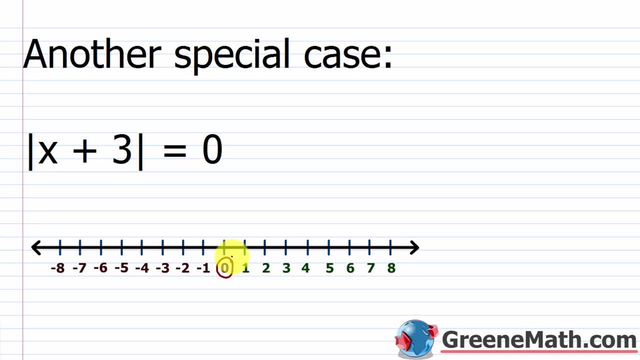 maps and I say: how far am I away from where I'm standing? I'm 0 units away. so it's a distance. it's 0 units away from itself. so in this case I would just say: well, if the absolute value of x plus 3 equals 0. 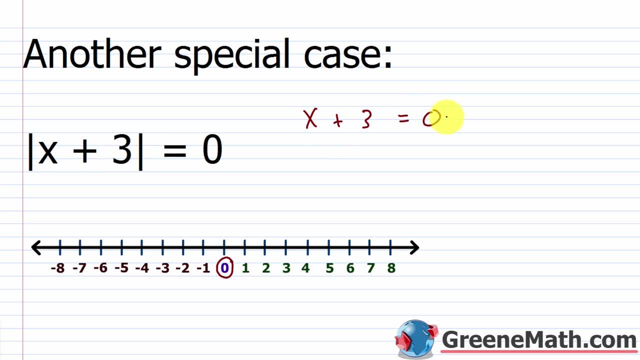 then I just solve one equation: x plus 3 equals 0. I don't need to go. x plus 3 equals negative 0. I see that on tests all the time too. please don't do that. there's no such thing as negative 0. negative 0 is just 0. 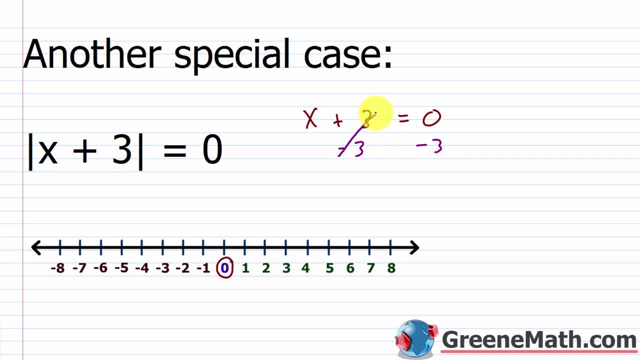 so then I would just subtract 3 away from each side here and I would get that x is equal to negative 3, and that makes sense, because if I plug in a negative 3 there, negative 3 plus 3 is 0. the absolute value of 0 is 0. 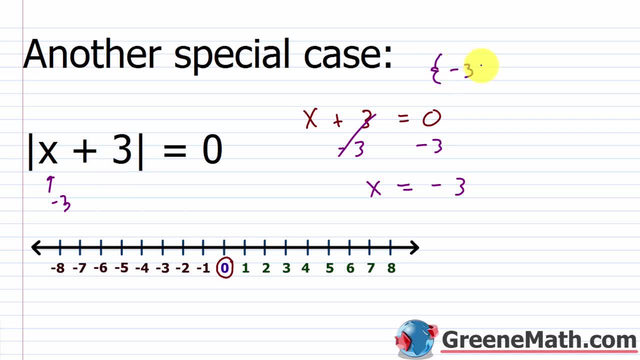 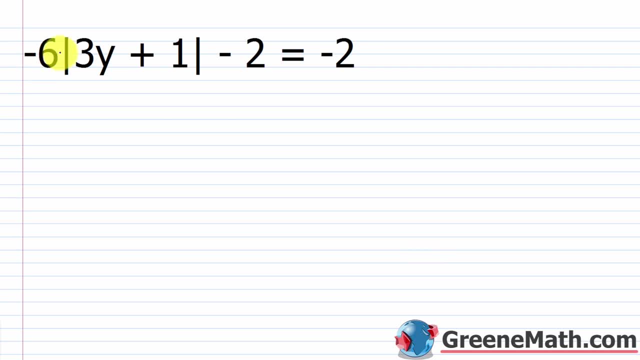 and we could just write this again using solution set notation: put a negative 3 inside of some set braces, alright, so let's look at an example here. so we have negative 6 times the absolute value of 3y plus 1 minus 2 is equal to negative 2. 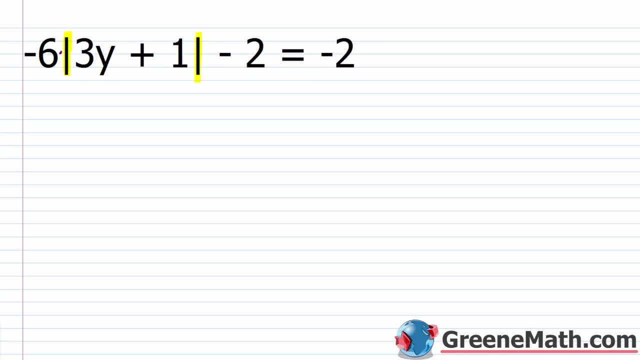 again, let me isolate my absolute value operation and so to do that, I'm going to add 2 to each side, so that will cancel and I'll have negative 6 times the absolute value of 3y plus 1, and this is equal to negative. 2 plus 2 is 0. 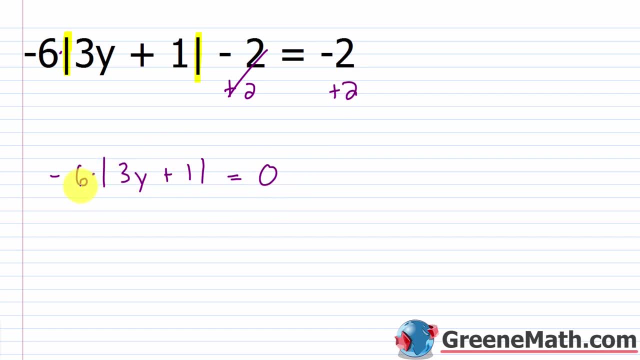 now I want this by itself. if negative 6 is multiplying that divide both sides by negative 6 to get rid of it. ok, this is going to cancel with this and I'll have the absolute value of 3y plus 1 is equal to 0 over negative 6 is 0. 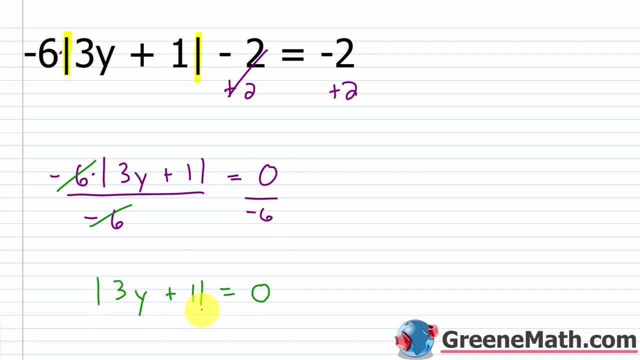 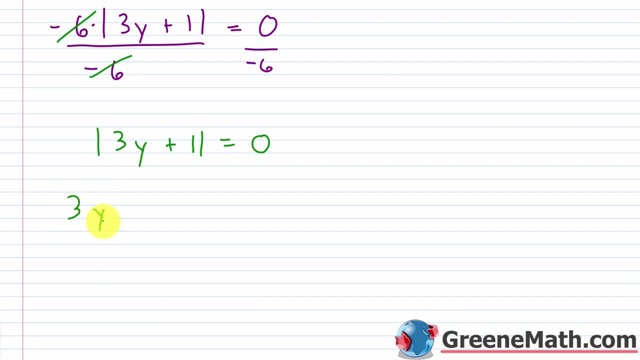 I have the scenario I just told you about: the absolute value operation is isolated and it's equal to 0. so there's only one possibility. it can only be true that 3y plus 1 equals 0. again, please don't say, or 3y plus 1 equals negative 0. 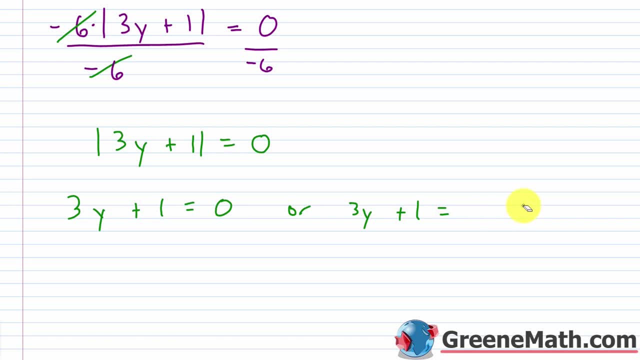 the negative or opposite of 0 is just 0. so you have one situation here to solve and I just subtract one away from each side, I'll get 3y equals negative 1. divide both sides by 3 and I get y equals negative 1. third, 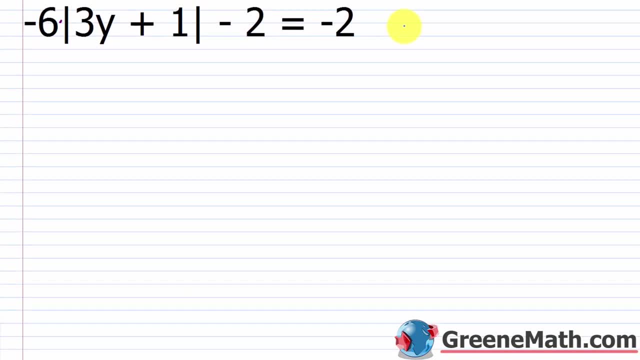 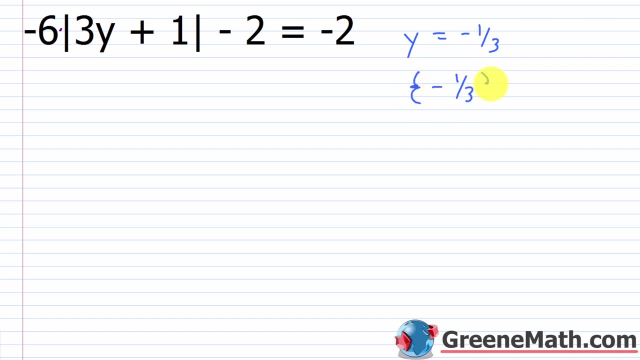 ok, so let's erase everything. ok, so y equals negative 1 in solution set notation. I put a negative 1 third inside of some set braces and again, if you want to check this, pause the video, plug in a negative 1 third here and see that you get a true statement. 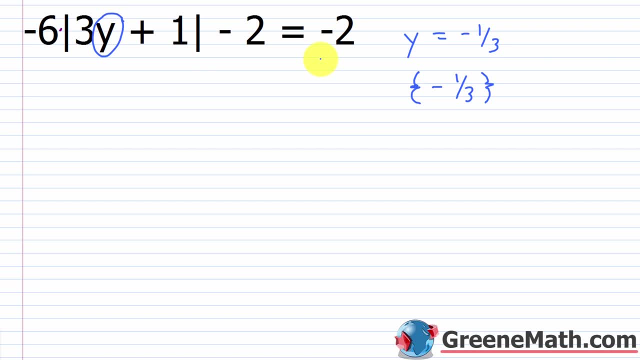 you should get: negative 2 equals negative 2, and in fact let's just go ahead and do it, so I'll have negative 6 times the absolute value of 3 times negative 1, third plus 1, and this is minus 2- equals negative 2. 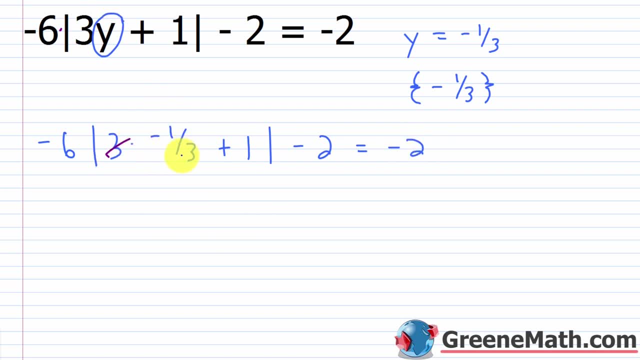 so 3 times negative 1. third, this will cancel with this and give me negative 1. negative 1 plus 1 is 0, so this right here would end up being 0, so I'd have negative 6 times. remember this is multiplication, because it's hanging out outside. 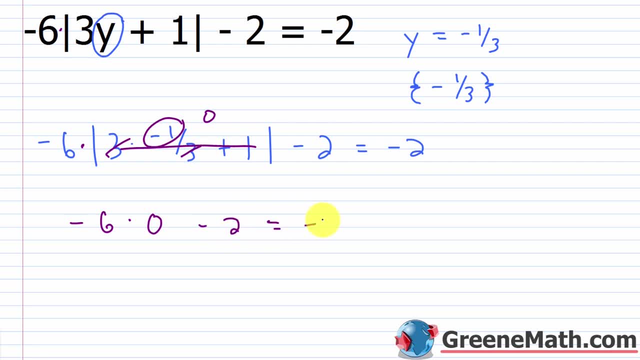 I'd have negative 6 times 0, then minus 2 equals negative 2 0 times. anything is 0. so this is gone, this is 0. I'll just have negative 2 equals negative 2. so yes, this solution is correct: y equals negative 1. third, 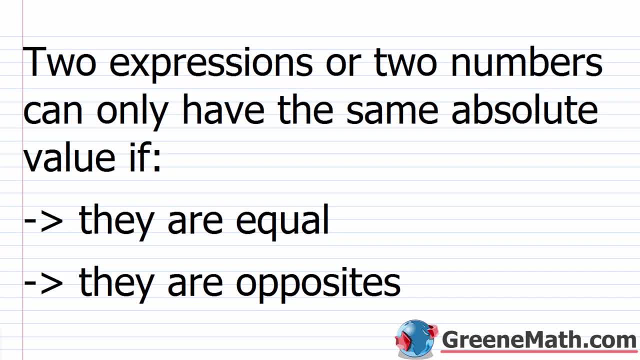 alright, so kind of the last special case scenario you're going to deal with is where you have two absolute value expressions that are equal to each other. so before we kind of get into that, I want to remind you of one thing that you might have overlooked. so two expressions. 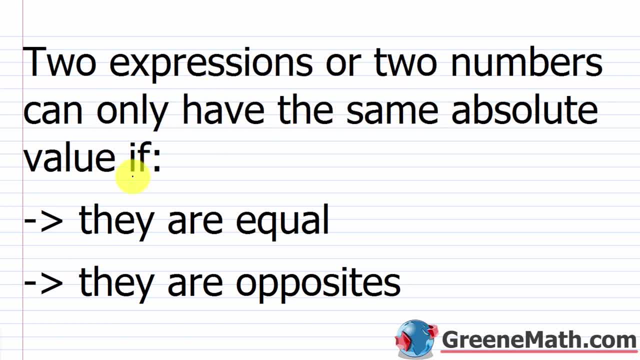 or two numbers can only have the same absolute value if they are equal. so that's one scenario: 2 has the same absolute value as 2, those two numbers are the same, they're equal. negative 2 has the same absolute value as negative 2, again, those two. 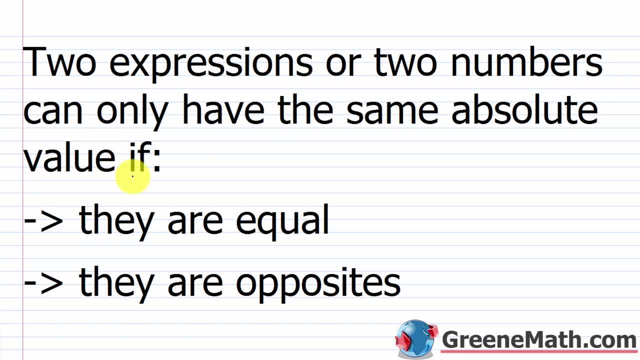 are the same. they're equal. negative 19 and negative 19 have the same absolute value or the other scenarios. they're opposites, like we've been talking about. so 14 and negative, 14, 12 and negative 12, 210 and negative 210. 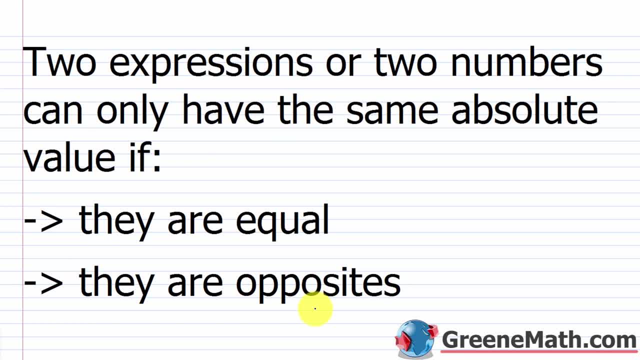 so they have the same absolute value because they're opposites. or again, numbers or expressions that are the same or equal also have the same absolute value. so those are your only two scenarios. so when we encounter something like this, the absolute value of 5x minus 3. 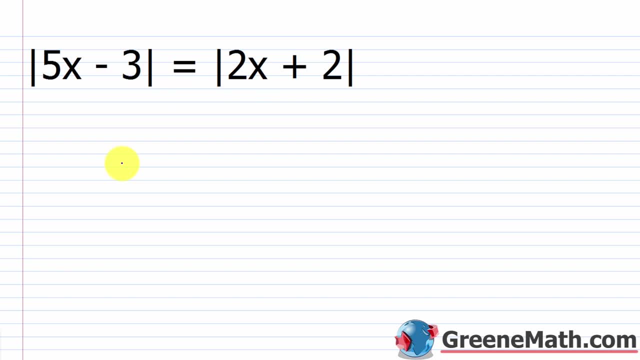 is equal to the absolute value of 2x plus 2. so there's two possibilities. one is that 5x minus 3 is equal to, or is the same as, 2x plus 2. so this would kind of be like saying the absolute value of. 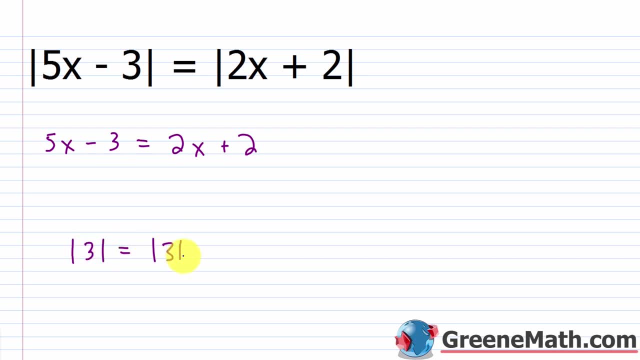 3 equals the absolute value of 3. they're the same same number, so of course the absolute value would be the same. we're saying that these are the same, so that's kind of your first scenario. then you have- OR you have- a second scenario. 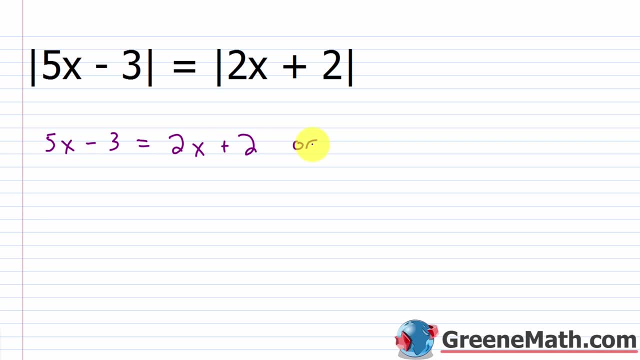 where you make one of these into its opposite. so, for example, I have: 5x minus 3 is equal to. if I want the opposite of this, I just put parentheses around it and I put a negative out in front. so the negative of or the opposite of. 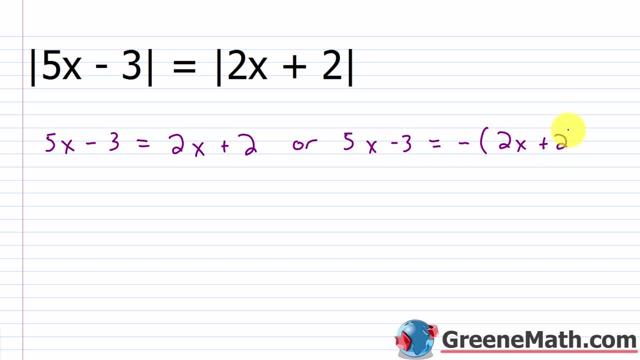 the whole expression. so 2x plus 2. the common mistake with this. a lot of people see it in their textbook and they forget about how it was modeled. they'll just put a negative out in front. this is only making the 2x negative. it's not doing anything with this. 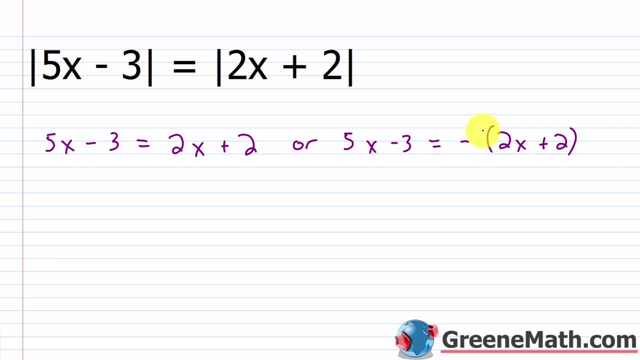 the whole thing. we've got to apply this negative there, so make sure you use parentheses there so you apply the negative to each term very important. so this here is the scenario where, let's say we have, the absolute value of 3 is equal to the absolute value of negative 3. 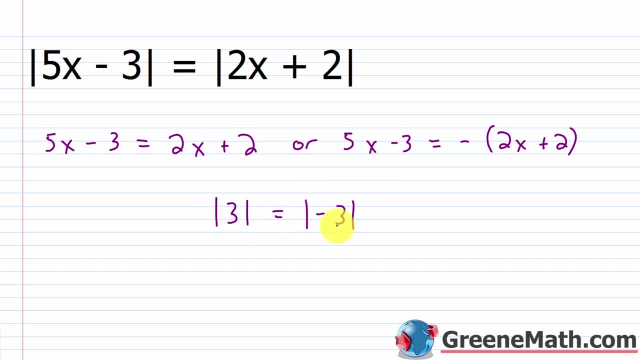 they're opposites, so they're still going to have the same absolute value. so we've covered each scenario again. two expressions can have the same absolute value: if they're equal or if they're negatives. here they're equal, here they're negatives. so we start out by solving this guy. 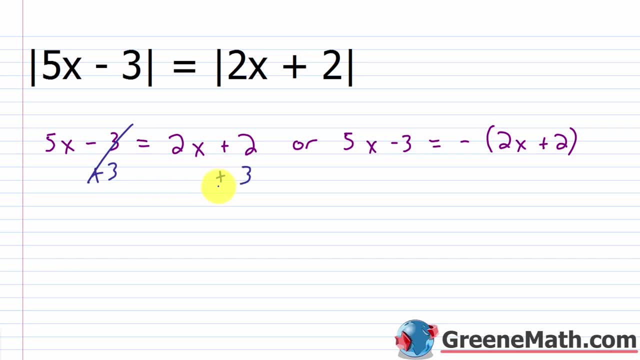 we add 3 to each side, that's going to cancel, and we subtract 2x away from each side, that's going to cancel. 5x minus 2x is 3x and this is equal to 2 plus 3 is 5. 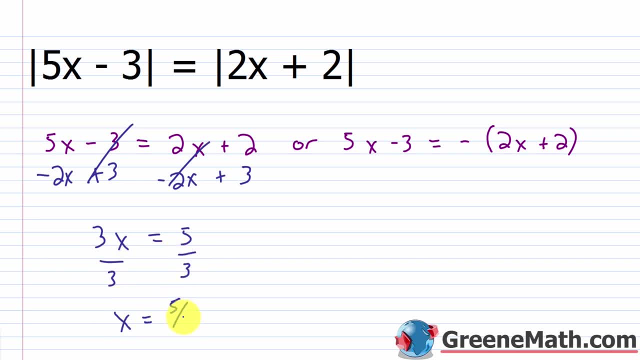 divide both sides by 3 and you get x is equal to 5 thirds. the other guy over here. let's distribute the negative to each term. just think about it as a phantom negative 1 out there. so we have, OR we will have 5x minus 3. 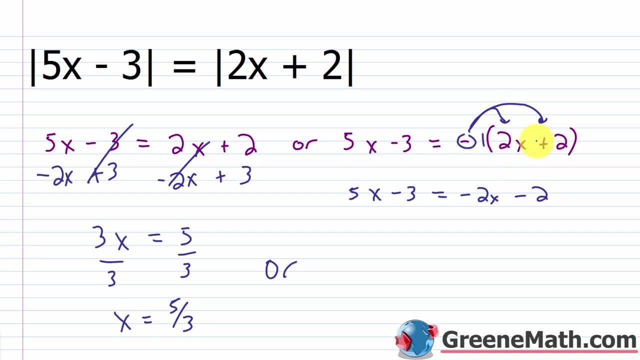 is equal to negative. 2x minus 2. just distributed the negative. let me add 3 to each side and let me add 2x to each side, so this will cancel and this will cancel. 5x plus 2x is 7x. 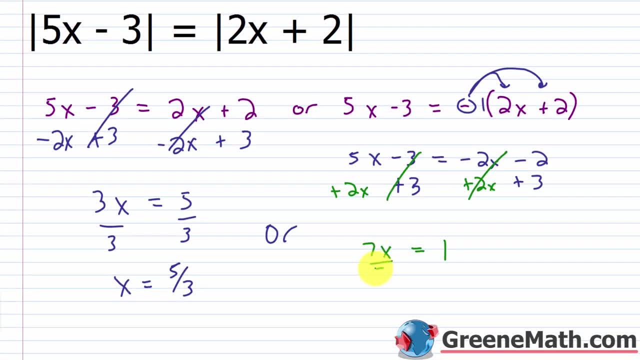 and this is equal to negative. 2 plus 3 is 1. divide both sides by 7 and we get that x is equal to 1 seventh. so my solution set here contains two elements. we'll have 1 seventh and 5 thirds, and let's go ahead and check this one. 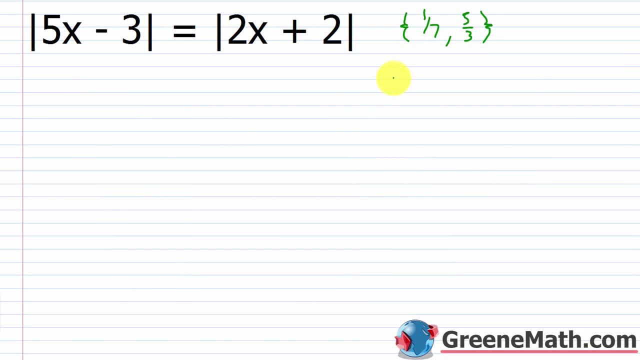 because I want you to see that it works. so again we have that x is equal to 1 seventh, or x is equal to 5 thirds, and if I start by plugging in a 1 seventh for x here and here, let's see what we get. 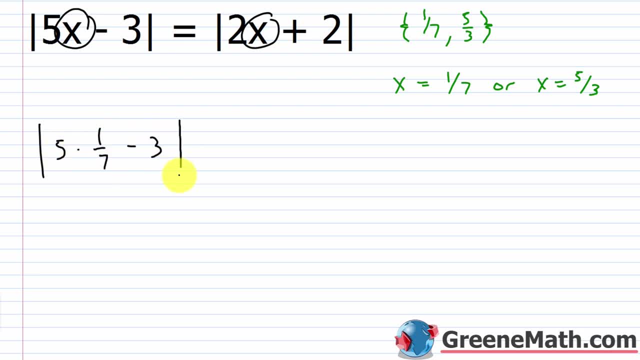 so we'd have the absolute value of 5 times 1 seventh minus 3. this should be equal to the absolute value of 2 times 1 seventh plus 2. so 5 times 1 seventh is 5 sevenths. let me just replace this in here. 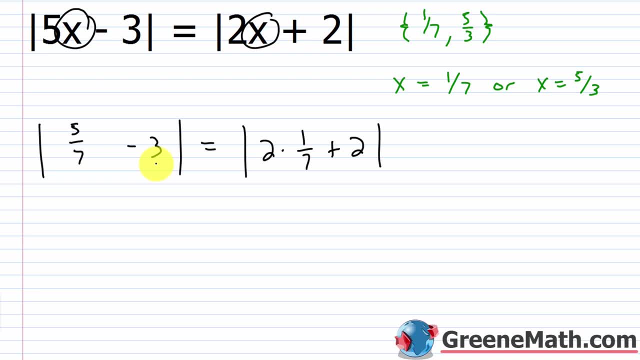 and this is minus 3, so I've got to get a common denominator going. multiply 3 by 7 over 7, I'll have 21 over 7 and this ends up being negative 16 over 7, which, of course, once I take the absolute value of, would be 16 over 7. 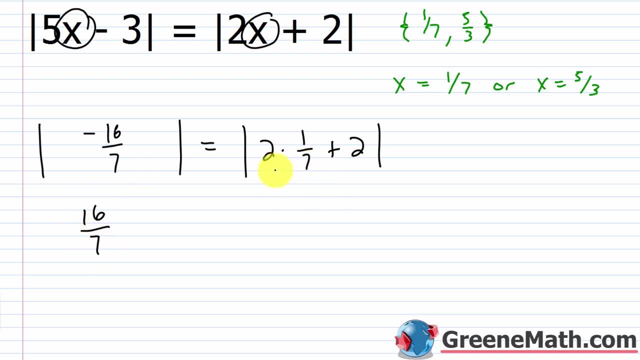 then over here I have 2 times 1 seventh plus 2. if I do 2 times 1 seventh, that's 2 sevenths. that's easy enough, and again I've got to get a common denominator going. so let's multiply 2 times 7 over 7. 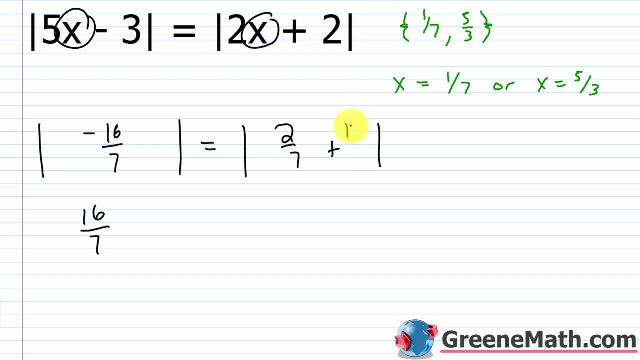 2 times 7 would be 14, so this would be 14 over 7. 2 plus 14 would be 16. so this is 16 sevenths and, of course, if I take the absolute value of that, that's just 16 sevenths. 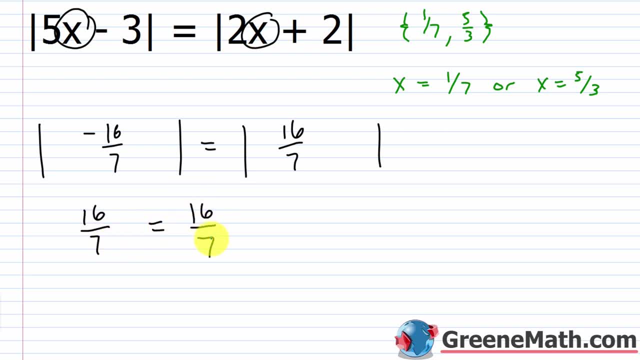 so I get 16 sevenths equals 16 sevenths. so we can see that the solution x equals 1 sevenths does work. we get the same value on the left and the right side. and again, remember this solution came from when we set them as negatives of each other. 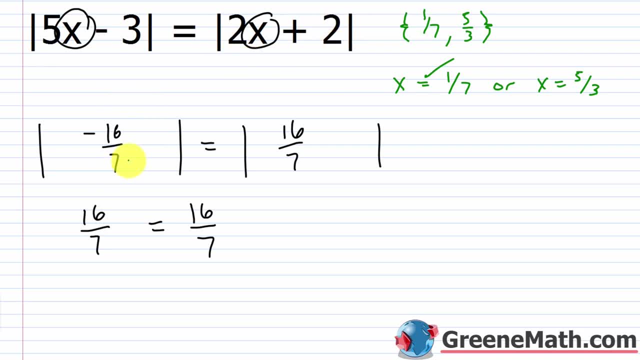 I took this one and I set it equal to the negative of this one. so you have a negative of this one, but when we take the absolute value, it's the same value. so, again, that's why it works out. now for the next part, let's check the other guy. 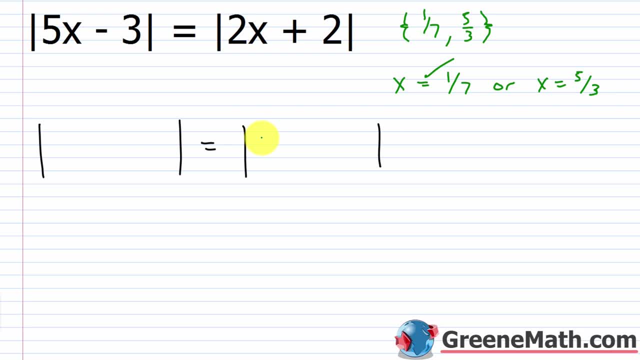 we're going to put the same value on each side in the absolute value operation, because we did this equals 0, without making one of them the negative of the other. so for the other one we have the absolute value of 5 times 5 thirds minus 3. 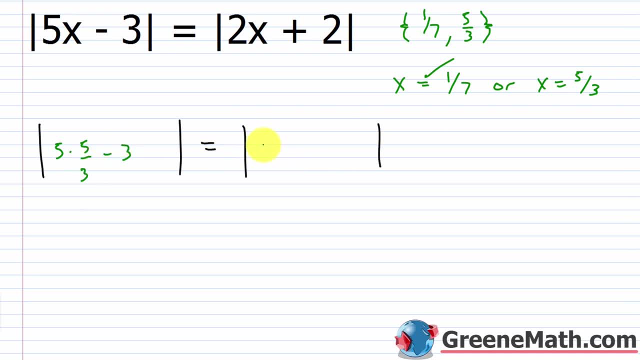 then this equals the absolute value of 2 times 5 thirds plus 2. so of course, 5 times 5 thirds. 5 times 5 is 25. so this would be 25 thirds. so to get a common denominator, multiply this by 3 over 3. 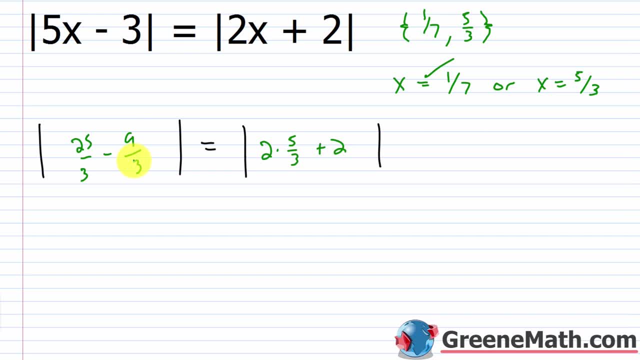 you would end up with 9 thirds. so 25 minus 9 is 16, so this would be 16 thirds. so it would be 16 thirds over here. 2 times 5 is 10. you'd have 10 thirds. so 10 thirds. 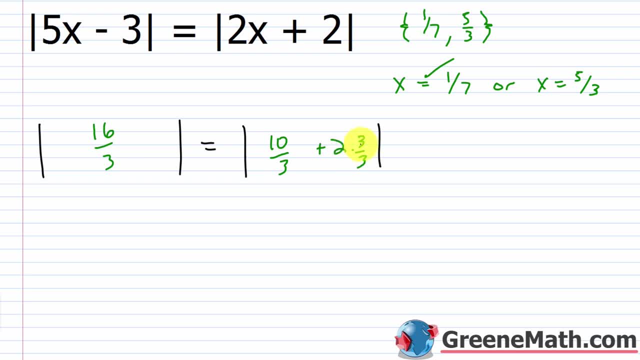 and over here to get a common denominator. multiply this by 3 over 3. 2 times 3 is 6. you'd have 6 thirds, and if you add 10 plus 6 you get 16 over the common denominator of 3. you'd have 16 thirds. 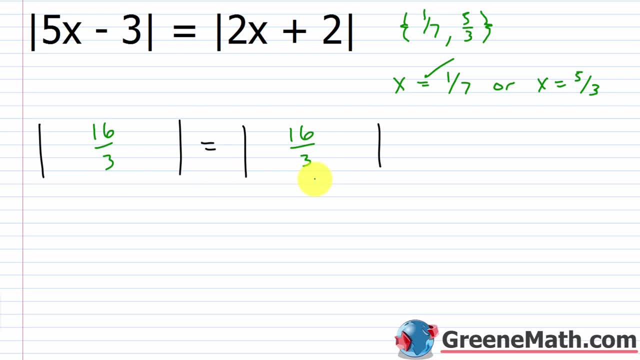 so the absolute value of 16 thirds is equal to the absolute value of 16 thirds. of course, that's true. you get 16 thirds equals 16 thirds. so yes, this one works out as well. this solution came from us just saying: 5x minus 3 equals 2x plus 2. 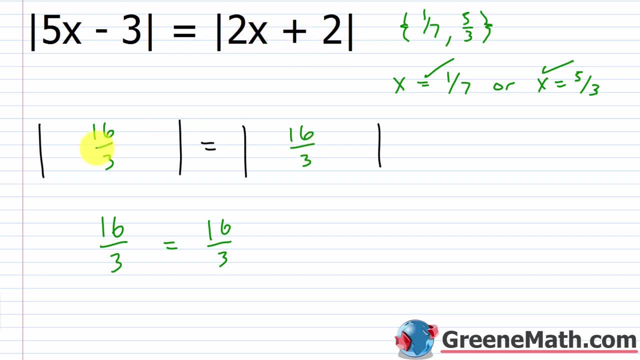 so, of course, when we got down to this stage of checking it, it's the same value in here as in here. it's the same value that we're taking the absolute value of in each case. again, when we checked this one, we had the negatives of each other. 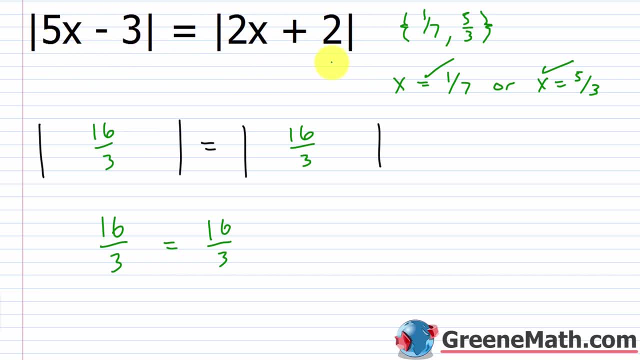 because we said 5x minus 3 is equal to the negative of this expression, 2x plus 2, and so that's why we ended up with this equals the negative of this, but again, when we take the absolute value, it makes everything positive, so that's how we got a true statement in that case. 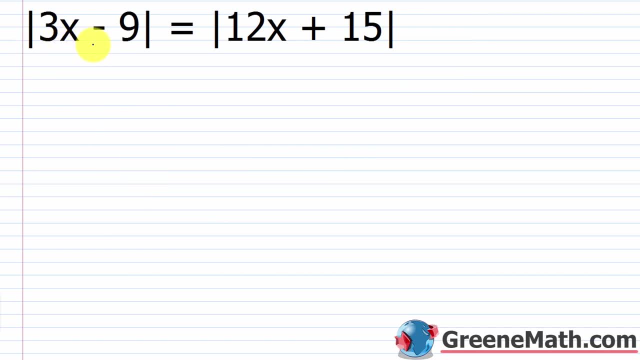 alright, let's take a look at one more. so the absolute value of 3x minus 9 is equal to the absolute value of 12x plus 15. so again, I want one scenario where they're equal to each other. so 3x minus 9. 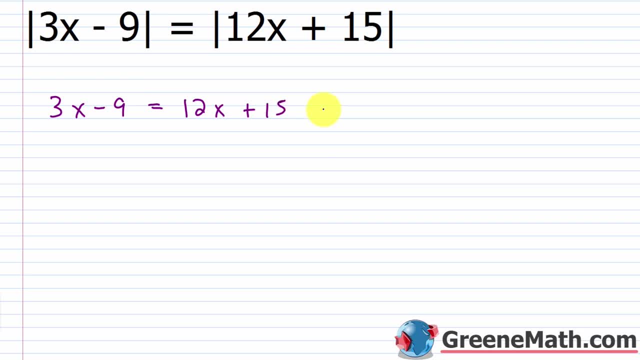 is simply equal to 12x plus 15. or I want another scenario where they're opposites, so I can make this guy 3x minus 9. I can make it negative. so the negative of that whole thing- again, make sure you use parentheses- is equal to. this would stay positive. 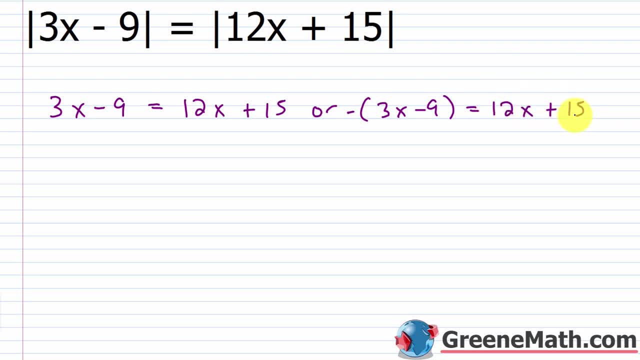 so 12x plus 15. alright, I won't do anything to that, it just stays as it is. so this is just straight. removing the absolute value bars this one, I'm making one and two its opposites, so that we follow the rule to say: if two numbers, 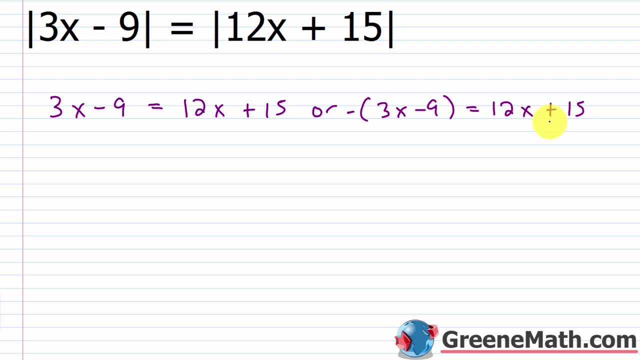 or two expressions have the same absolute value. they're equal to each other, or they're negatives. equal, they're negatives. ok, let's solve each one. so we add 9 to each side over here and we subtract 12x from each side, and so this cancels. 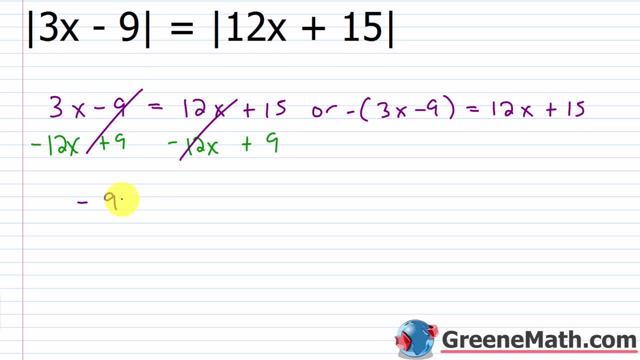 and this cancels. 3x minus 12x is negative 9x and this equals 15 plus 9 is 24. we divide each side by negative 9 and this will cancel. we'll get x is equal to 24. over negative 9 is going to be negative. 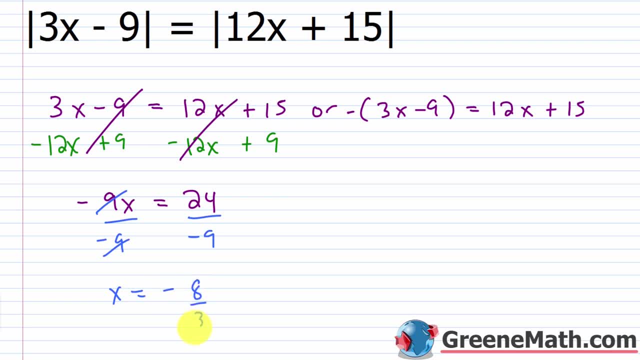 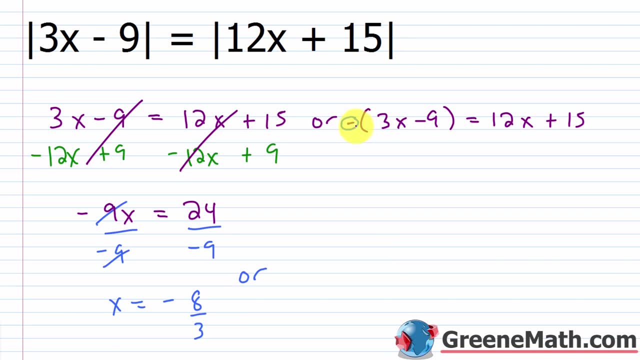 and each is divisible by 3, so this would be negative 8 over 3, so negative 8 thirds. then we have or? alright, let's deal with this scenario now. so the first thing I'm going to do is just apply the negative, so negative times 3x is negative 3x. 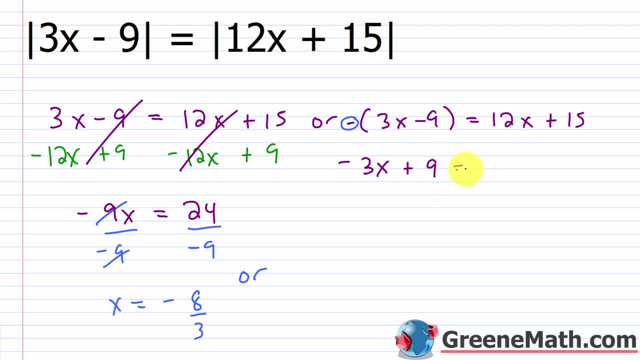 and then negative times. negative 9 would be positive 9. this equals 12x plus 15. now what I'm going to do is subtract 9 from each side of the equation and I'm also going to subtract 12x away from each side of the equation. 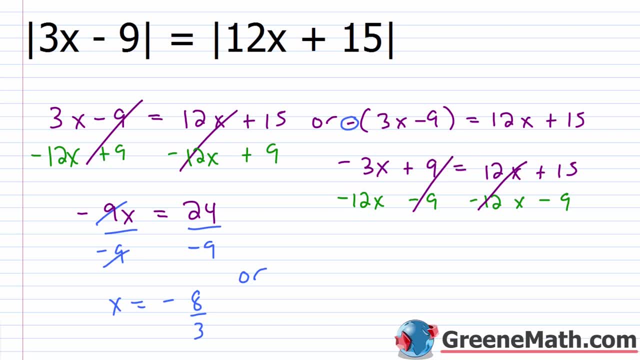 so what's going to happen is: this will cancel, and this will cancel. negative 3x minus 12x is negative 15x, and this equals 15 minus 9, which is 6. now all I need to do is divide both sides by negative 15. 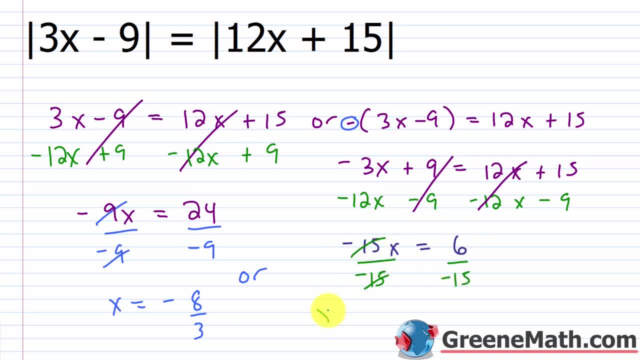 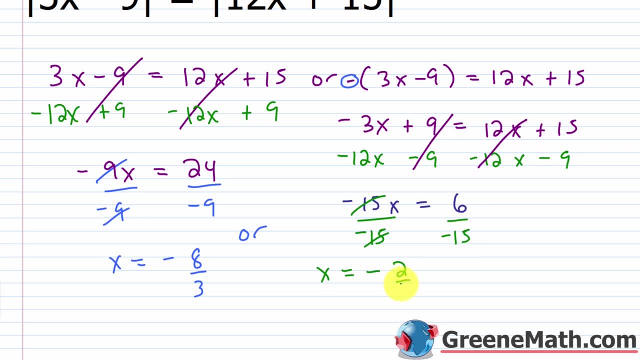 this cancels with this and I've got. x is equal to each is divisible by 3. I know it's negative. 6 divided by 3 is 2, 15 divided by 3 is 5. so this is negative 2 fifths. so x equals negative 8. 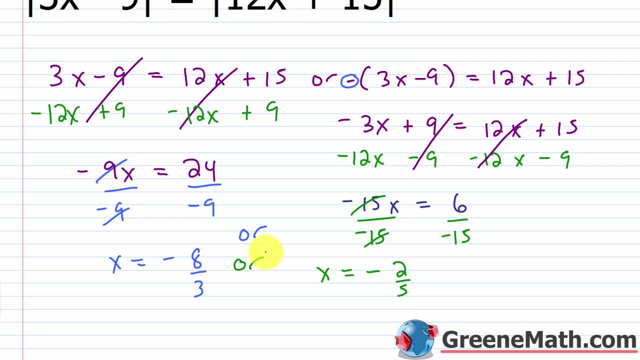 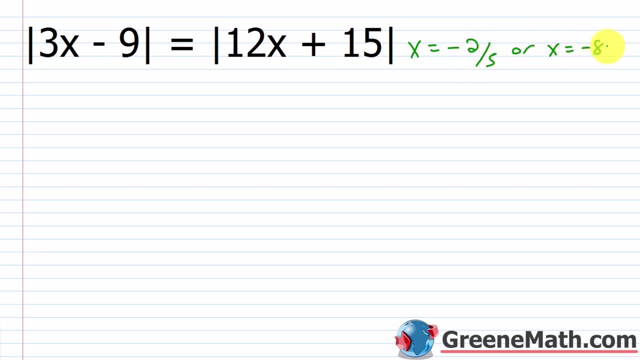 thirds, or x equals negative 2 fifths. so let's write that up here. so again, x equals negative 2 fifths, or x equals negative 8 thirds. and again in solution set notation we can write this as negative 8 thirds, comma negative 2 fifths. 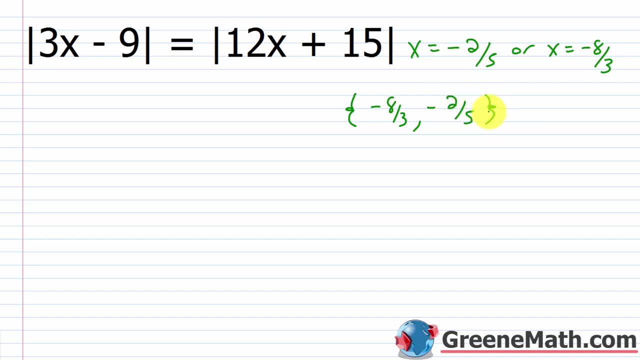 inside of some set braces, and I'm not going to check this, I'm going to leave this up to you to check again. you're going to plug in each value for each occurrence of x. so I'd plug in negative 8 thirds here and here I would evaluate and make sure I get the same. 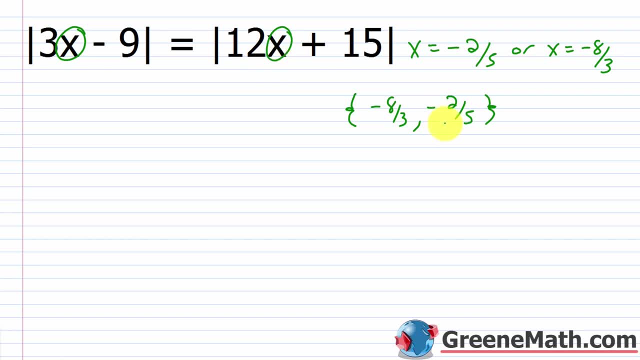 value on the left and the right, and I'm going to do the same thing with negative 2. fifths, what you're going to find is that in one scenario, you'll have the same value inside the absolute value operation on each side. that makes sense because for one of these, 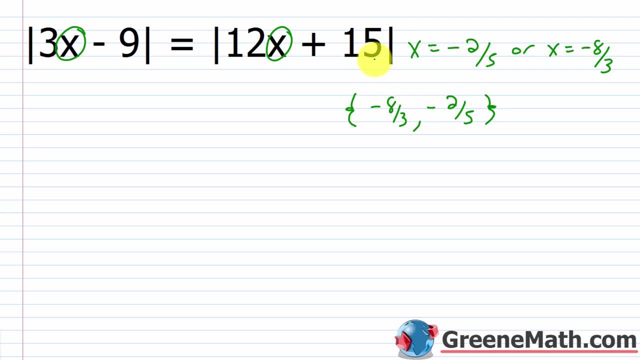 we just said: remove the absolute value bars. 3x minus 9 is equal to 12x plus 15. so that's what we expect there. in the other scenario we said the opposite of this was equal to this. so in that scenario, when you check, 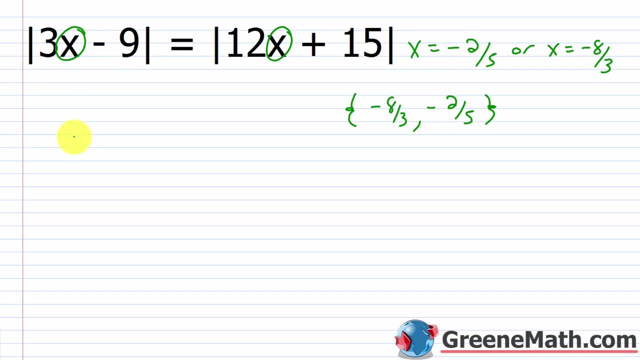 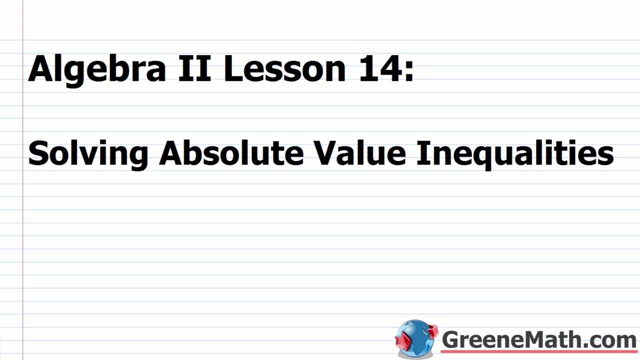 you're going to end up with opposites inside of the absolute value operation. when you take the absolute value, you'll end up with the same value on each side. hello and welcome to algebra 2, lesson 14. in this video, we're going to learn about 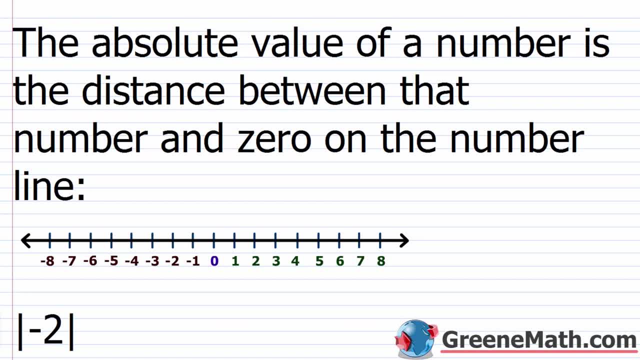 solving absolute value inequalities. so in our last lesson we learned how to solve an absolute value equation. so here we're just going to take the next step and learn how to solve an absolute value inequality. this isn't any more difficult and the reasoning is the same. okay, so the main. 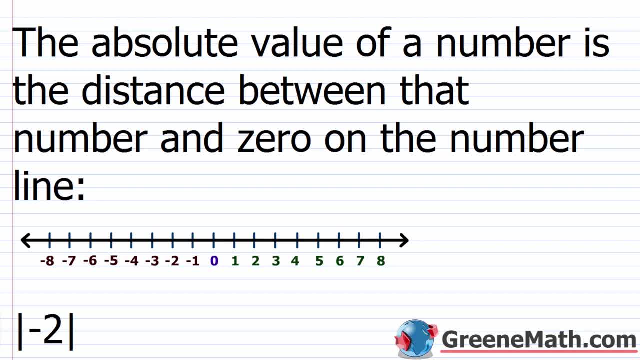 thing I want to make sure that you understand, in case you didn't watch the last lesson, is the concept of absolute value. it's very, very basic, but if you don't understand it, you'll have a hard time understanding the structure of these problems. so, the absolute value of a number. 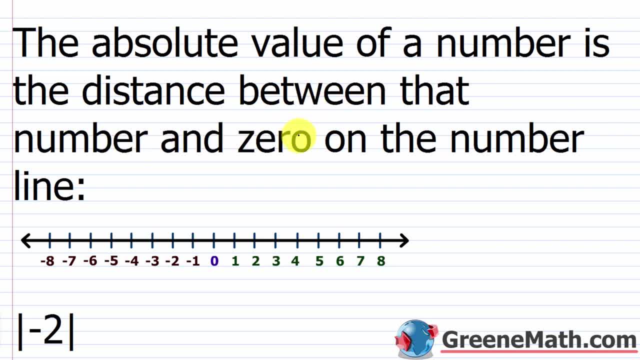 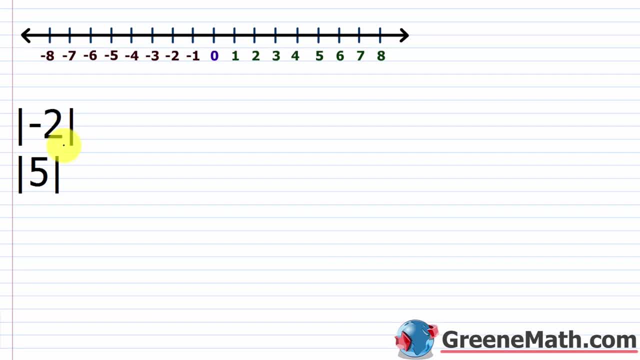 is the distance between that number and zero on the number line. so I have here a sample number line and I just have two quick examples of absolute value. so we know that if we see a number inside of these vertical bars that means we want to find the absolute value of it. 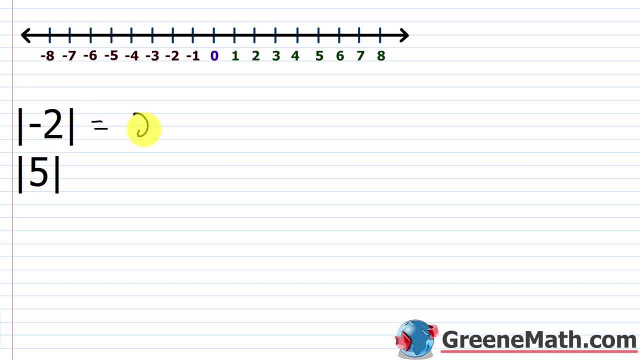 so the absolute value of the number negative two is just two, and so we know that. from the number line we can see that negative two is here and zero is here, and so what I can do is I can count how far away negative two is from zero. it doesn't matter. 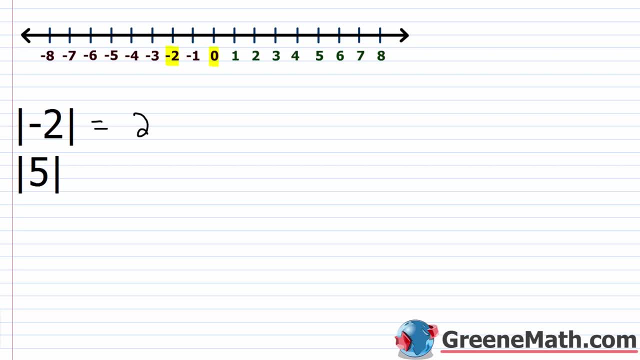 the direction I move. it's just how many units I'm going to move. so we would travel one, two units. so you get from negative two to zero. so my absolute value is two and we all know at this point that if you take the absolute value of a positive number, 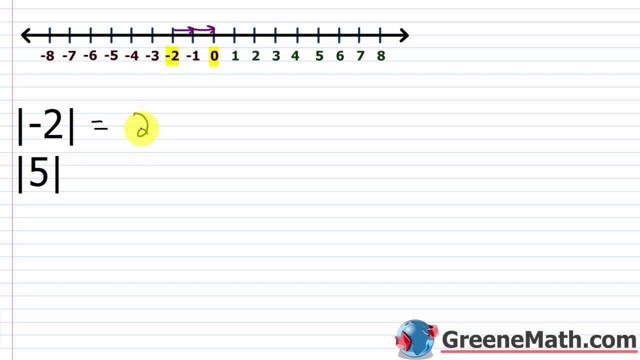 it's just that number. if you take the absolute value of a negative number, you just make it positive. so here I took the absolute value of negative two, just made it positive. so for the absolute value of five I just keep the number right. it's just five and again. 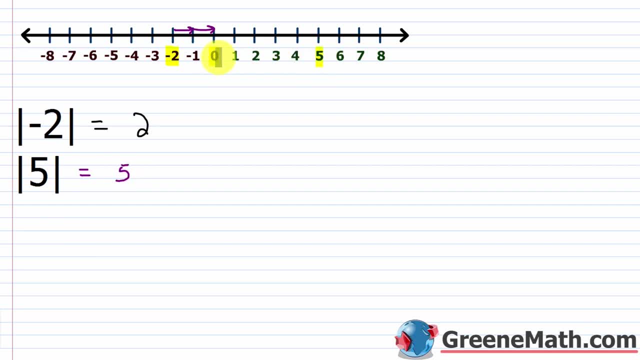 you can demonstrate this on the number line: here's five and again here's zero. and I would go one, two, three, four, five units to get to zero. and again, it doesn't matter which direction I go, we're just counting distance. it's just the same thing as. 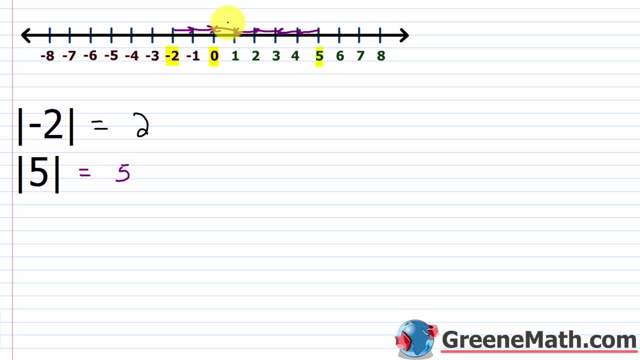 if you get in your car and you ask your GPS how many miles you have to go to a certain location, well, let's say, as this example goes, it's fifty miles. and let's say I'm in a different location now and it's exactly fifty miles away. 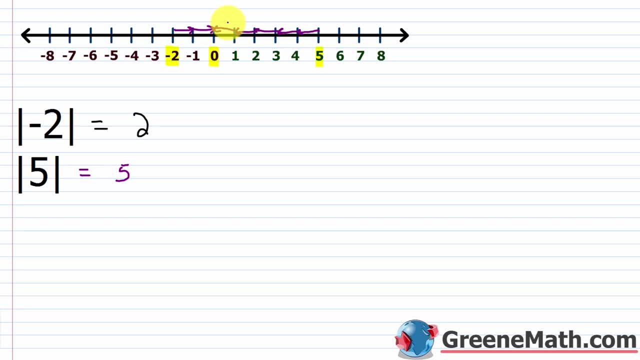 it would still tell me I'm fifty miles away. it wouldn't say it's negative fifty miles now, or it wouldn't change based on the direction I'm coming from. fifty miles is fifty miles doesn't matter which way I'm coming from, so it's the same concept here. 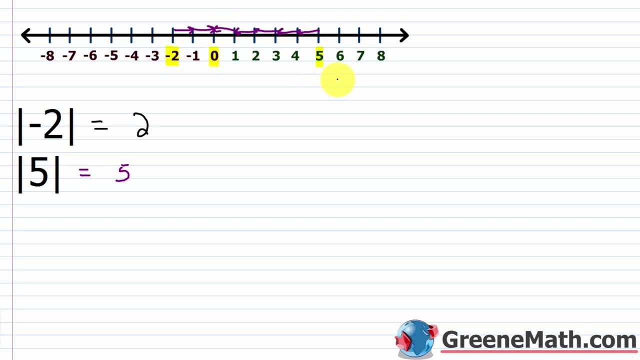 so absolute value can never be negative. it's a distance, so it's got to be zero or positive. and I think about this with driving again. if I tell you we've got to drive somewhere today, we can either say: nah, I don't feel like going, and we drive zero miles. 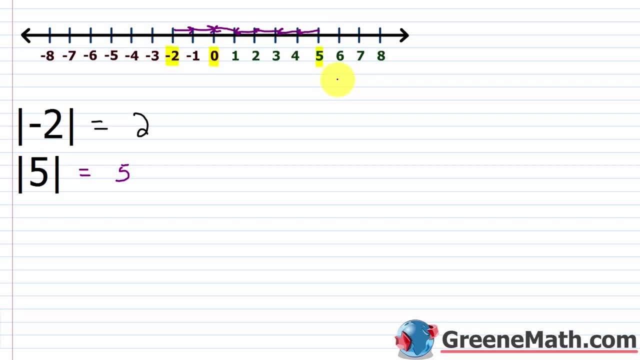 or we can drive some positive amount, but we can't not go somewhere or drive backwards or something silly like that and come up with a negative distance. okay, it just doesn't work that way, alright. so now that we understand the concept of absolute value, let's look at a very simple problem. 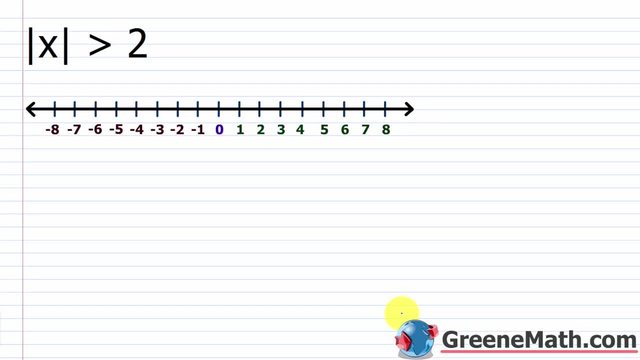 alright, so let's take a look at our first sample problem. this is a very easy one that you'd see at the very beginning of the section, and it's just to understand what's going on when we're asking these questions. so the absolute value of x is greater than two. 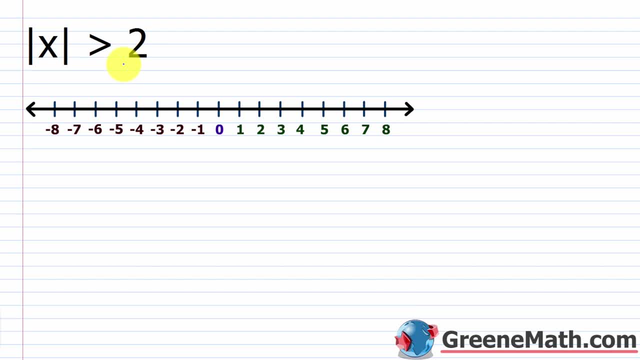 what are we asking for? you might want to pause the video and just think about that for a second. what are we asking for? well, we're asking for values whose absolute value is greater than two. or, if I started at zero, what value are more than two units away from zero? 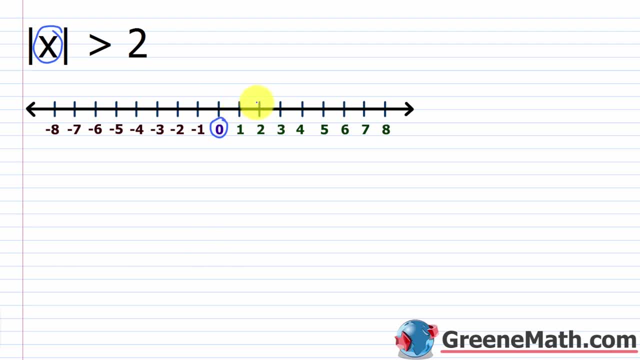 on the number line. well, if I just go one, two in this direction, I know that anything larger than two would work, so I'd shade everything to the right here. and if I go one, two units to the left, I know anything less than negative two would work, so I'd shade. 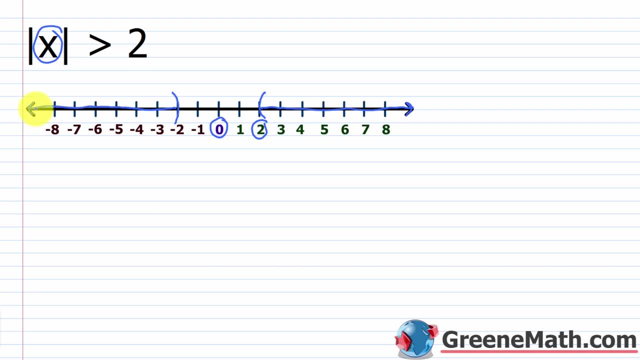 everything to the left here. so that gives me two solution sets: one where it's negative, infinity up two, but not including negative two and it's the union of this with this other guy, anything larger than two. so, thinking about this, any number that's involved in either solution set. 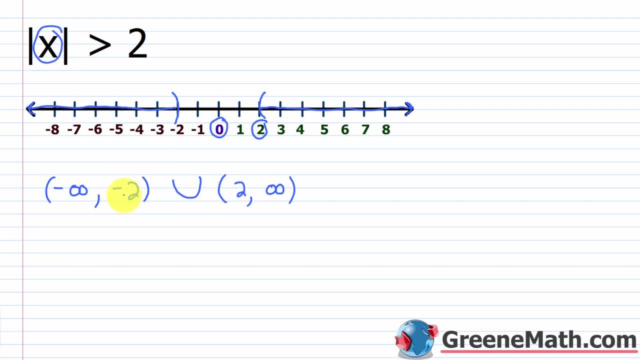 here would satisfy this inequality. just pick a number. let's say we pick negative eight. plug in a negative eight there. take the absolute value, you get eight. eight is larger than two. let's say you pick three over here. take the absolute value of three, you get three. three is larger. 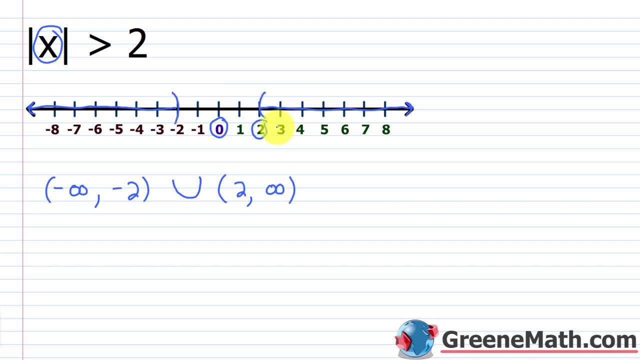 than two. the only numbers that won't work are from negative two to two, including both. if I plugged in a negative two there, the absolute value of negative two is two. two is not greater than two. that's false. so we know that this wouldn't work and this wouldn't. 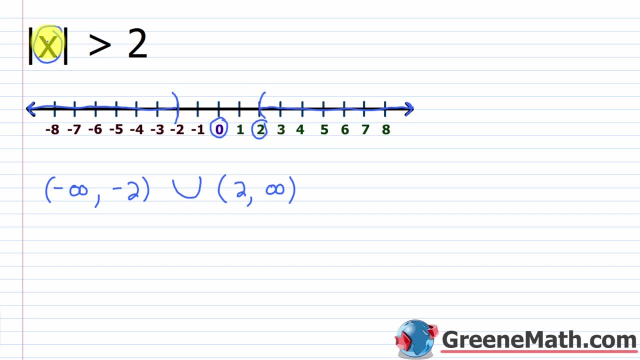 work and anything in between wouldn't work. if I chose one, the absolute value of one is one. one is not greater than two. so for this type of problem, where we see a greater than, we're going to end up with whatever's inside the absolute value bars. so 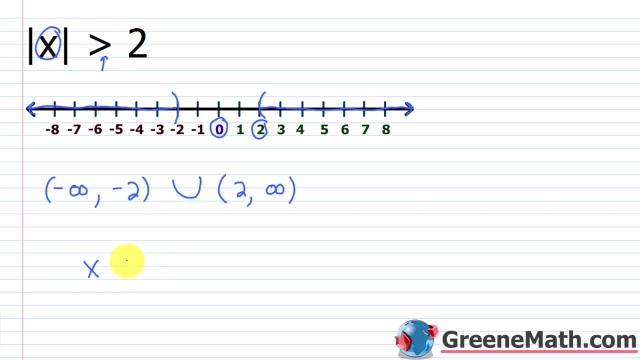 in this case it's x, and it's going to be greater than two. so in the first situation you would just remove the absolute value bars. that's your scenario. x is greater than two, then you're going to have an, or so it's going to be a. 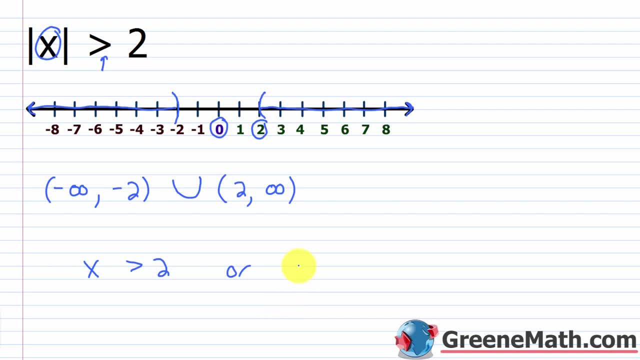 compound inequality and in the second situation you're going to flip the direction of the inequality. so I would have x. I'm going to flip this and I'm going to make this part right here. whatever's on the right side negative. now you might say: where does this come from? 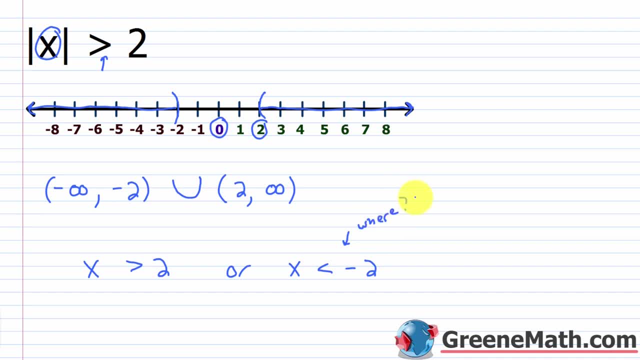 where- okay, that's a common question- you get in class because this one right here. this is very straight forward. everybody understands that x can be greater than two. that makes sense. but for x to be less than negative two, yeah, you can see it here. once you kind of think about it, it makes sense. 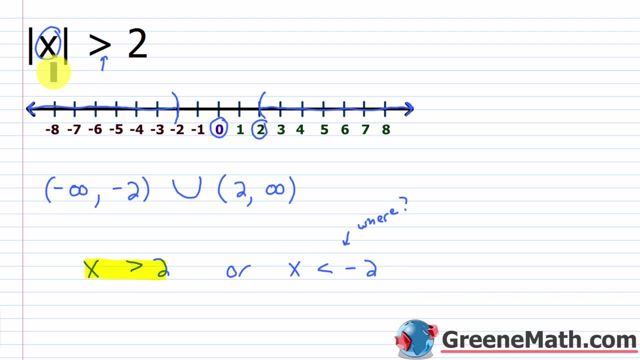 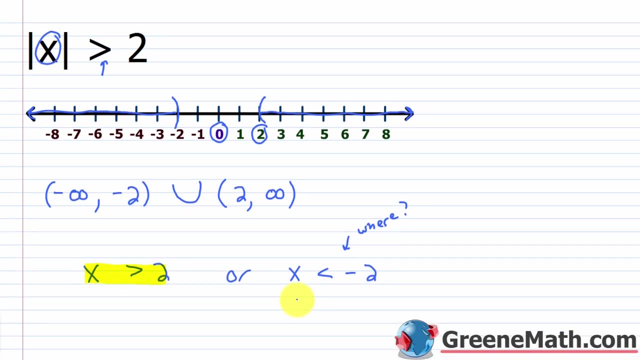 but once you get to the next example, it's like: where did that come from? well, all you'd have to do is think about absolute value for a second. if x, let me kind of scroll down a little bit- remember, I'm plugging something into the absolute value operation. 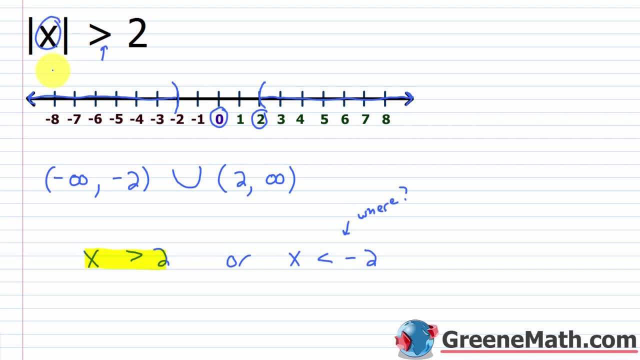 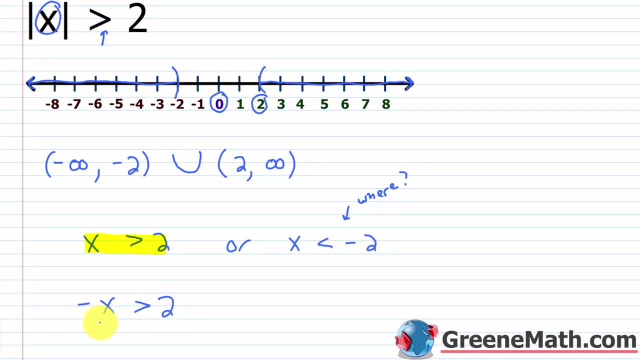 I can think about negatives as well, so the negative of x, the negative of x could also be greater than two, and if I divide both sides by negative one to get x by itself, what happens is I have to flip the direction of the inequality symbol, so this is going to become a less than. 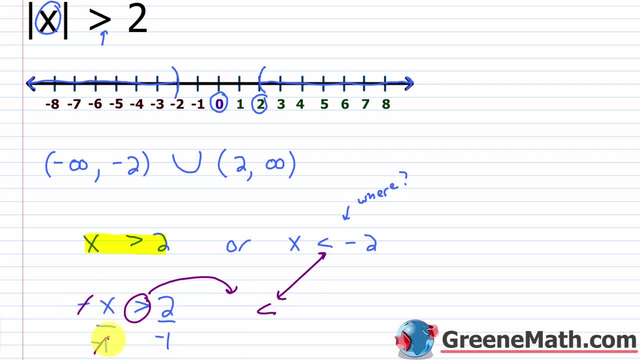 right, which is what I have there, and then this divided by this is just x, and then two over negative one is negative two. so that's where it comes from, and once you see me do that, you can remember to do that on your own in the next example. 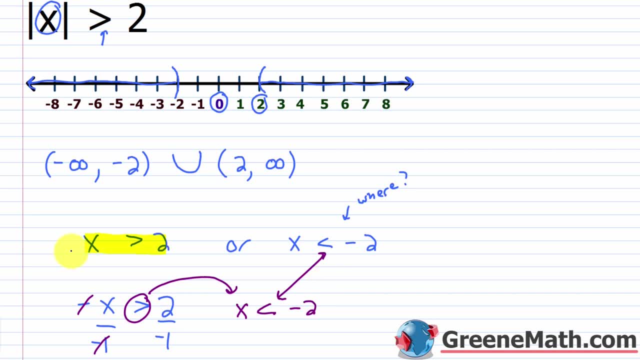 and then you won't have to think about what's the other scenario. this one's straightforward, this one everybody forgets, okay, so it's x is greater than two or x is less than negative two. if you had a generic example like the absolute value of x is: 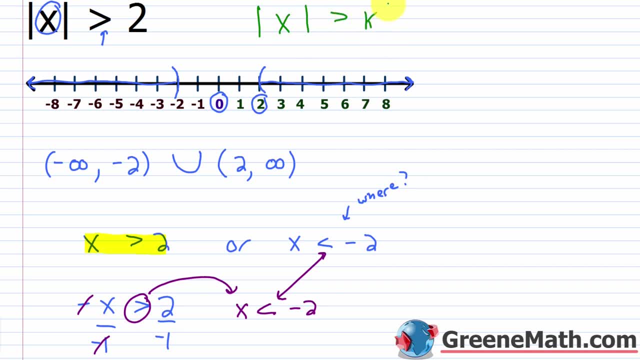 let's say greater than I don't know. let's say some variable k. well, this sets up to: x is greater than k or x is less than negative k. just following this format here, in this case k is just two. so x is greater than two or x is less than negative two. 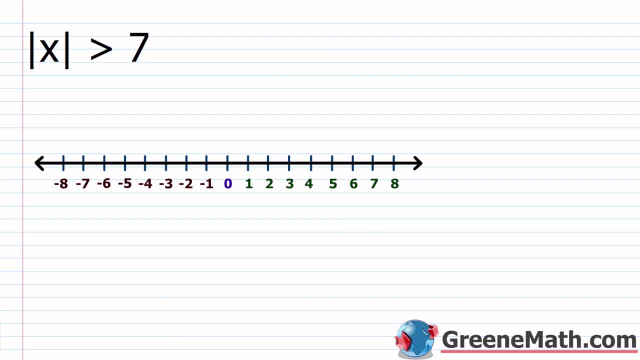 so here's another example, very similar we have: the absolute value of x is greater than seven. so again, what we're asking for here is: give me numbers whose absolute value or distance from zero is larger or greater than seven. well, I know, anything larger than seven would work. 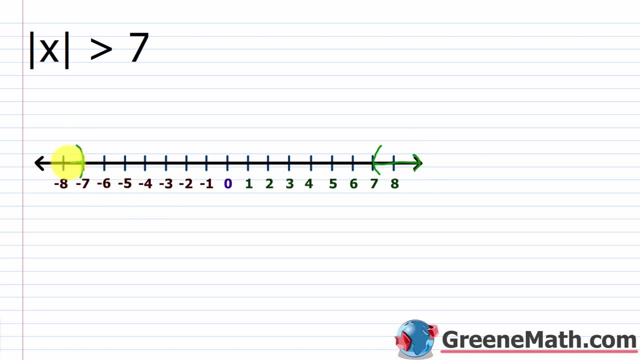 and also anything less than negative seven would work. because if I look at zero here, if I count one, two, three, four, five, six, seven, yeah, anything to the left of negative seven that works. and then again one, two, three, four, five, six, seven, yeah, anything to the right of seven. 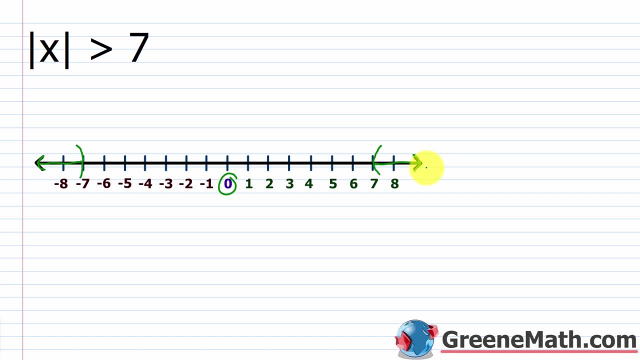 that works as well. that's a distance that's greater than seven units from zero. but again, we don't need to pull out a number line every time. if I have a greater than remember, use your generic example. the absolute value of x is greater than k. that's up to x is greater than k. 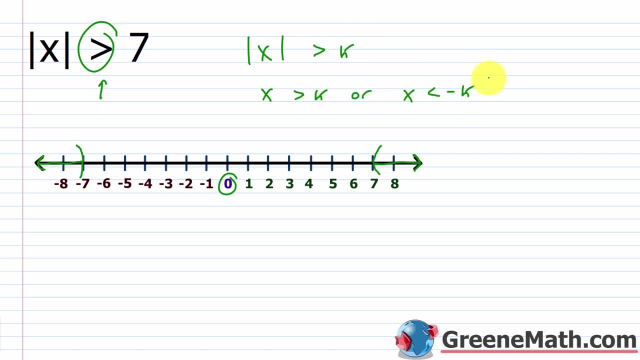 or x is less than negative k, so x could be greater than seven, or x could be less than negative seven. and again, let's do this one more time. where does this come from? well, I can take this part right here and say: well, the negative of x. 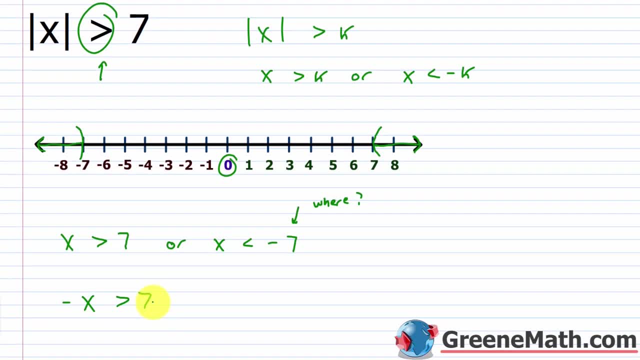 could also be greater than seven. the negative of x could also be greater than seven. I divide both sides by negative one. this gets flipped, and so you'd have this cancels out. x is less than negative seven. so that's where this came from, and again you might be asked to write this. 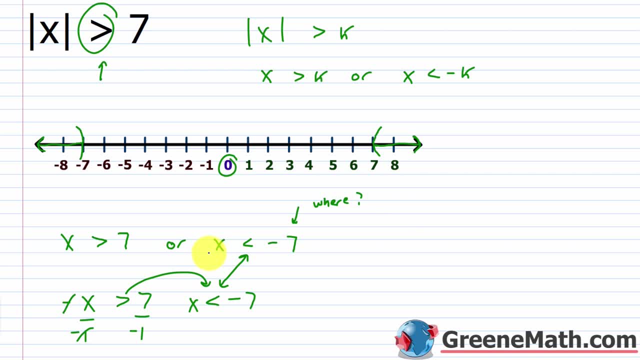 in interval notation and with, or it's the union of the two solution sets. so I would have: from negative infinity up to, but not including negative, seven and it's the union with the other solution set which is greater than seven out to infinity. alright, so now that we've dealt with the greater than scenario, 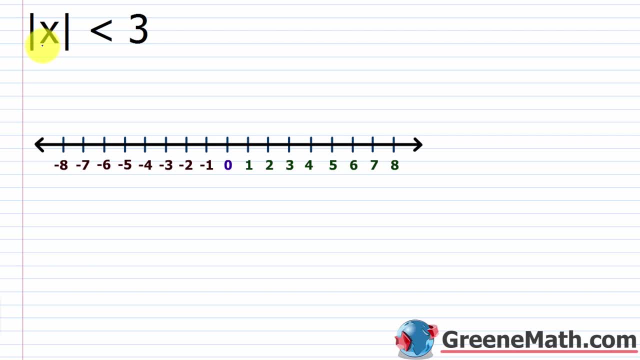 let's talk about the less than scenario. so we have: the absolute value of x is less than three. so here x can be any number that is less than three units away from zero, so anything less than one, two, three units. so it can't be three, but it can be anything less than. 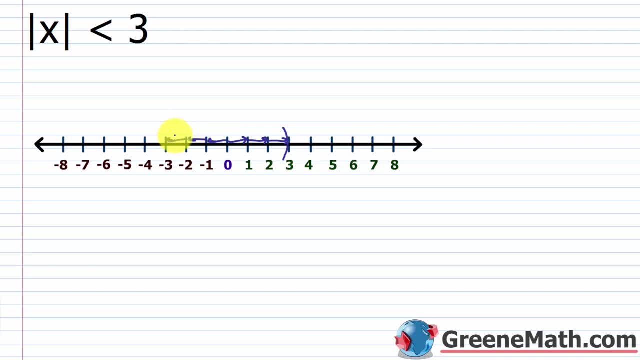 three. so one, two, three can't be negative three, but it can be anything greater than that. so basically, it's the numbers that are between negative three and three, shown here and again. the first scenario to do this, where x is just simply less than three, it's very straight forward: just remove the absolute. 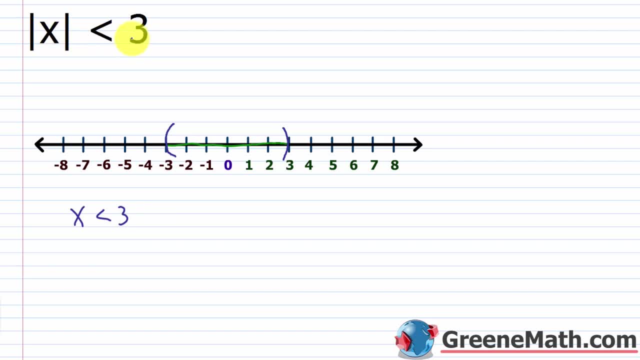 value bars and you have: x is less than three. for the other one, you have to think about the negative of x is less than three. well, if I divide both sides by negative one, what's going to happen is this gets flipped. this is now greater than this cancels with this. 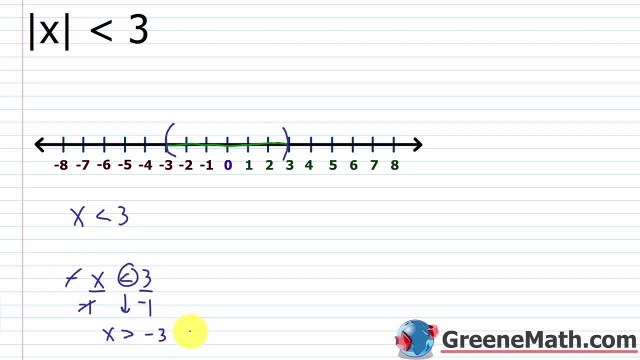 and I'll have. x is greater than negative three, so this sets up a compound inequality with and, and really you could write this as a three part inequality where x is in the middle, so x is going to be greater than negative three and it's less than three, so it's between: 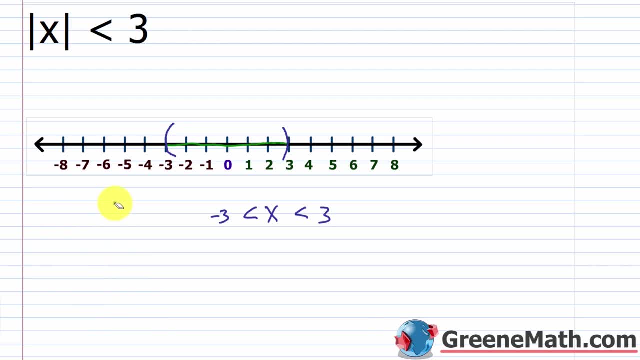 negative three and three and again. I'll just kind of erase this real quick. you could write something like this, an interval notation, pretty easily. you would put negative three next to a parenthesis comma three. so that's your solution set for this now, generically. if I had the absolute value of x, 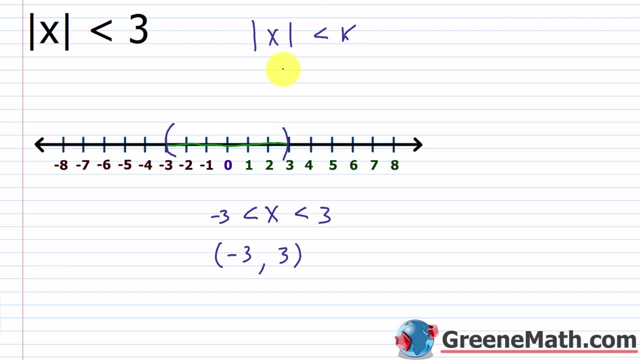 is less than k. what I want is remove the absolute value bars. you'd have x is less than k then, and you would also have remove the absolute value bars. you'd have x, flip the direction of this so you'd have greater than and make this negative, so negative. 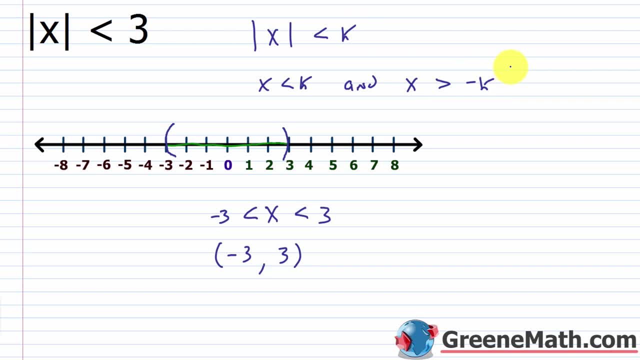 k. in each case, you basically do the same thing, but in one situation you have or, which is, when you have a greater than, and when you have a less than, you have an, and so let's take a look at the absolute value. of x is less than ten. 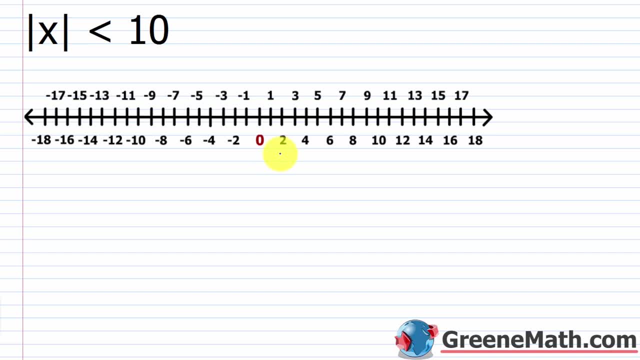 so, following our last example, we know that x would be what it would be, greater than negative ten and less than ten. see how fast I do that. so once you've got kind of the rules down, you can do these very quickly. but again, think about this as a concept. 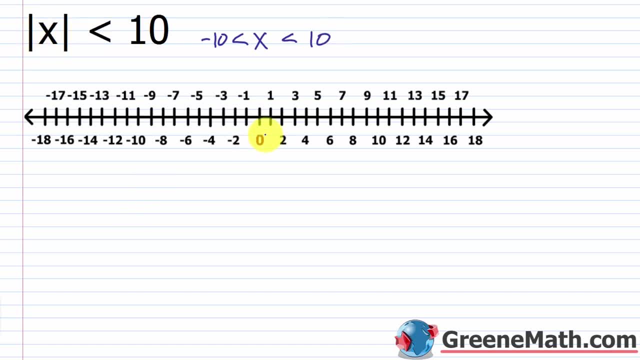 the absolute value of x is less than ten. so from zero, what's less than ten units away? well, we go to negative ten, and I would put a parenthesis facing to the right, because anything that is negative ten or further to the left wouldn't work their absolute value. 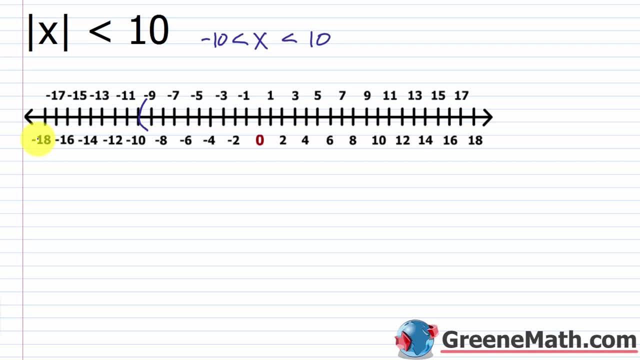 or their distance from zero is ten units or larger. I'm looking for less than ten, so, also going this direction, I would stop at ten. I'd put a parenthesis there, facing to the left. again, anything that's ten or larger won't work because the distance from zero is ten or more. 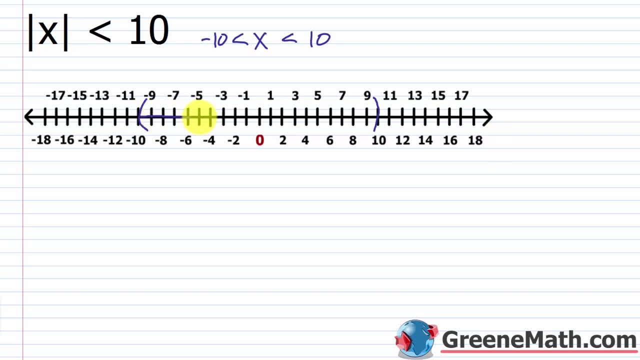 we want ten or less, so then we want all the values in between. here again, x can be larger than negative ten or less than ten. so in interval notation I would just simply write a negative ten comma ten, with a parenthesis next to each and again. just to go through this one more time. 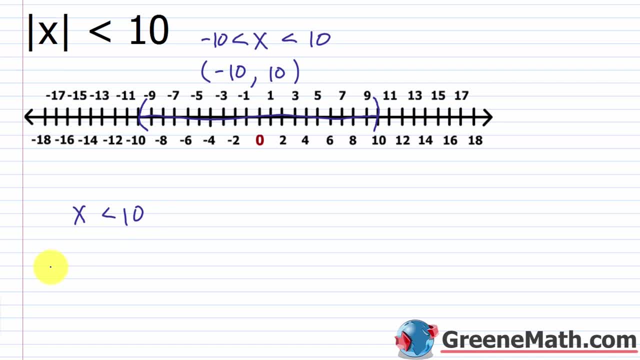 we know that x could be less than ten. the other scenario is the negative of x could be less than ten. we divide both sides by negative one. this flips and we end up with x is greater than negative ten. so this sets up the compound inequality: x is less than ten. 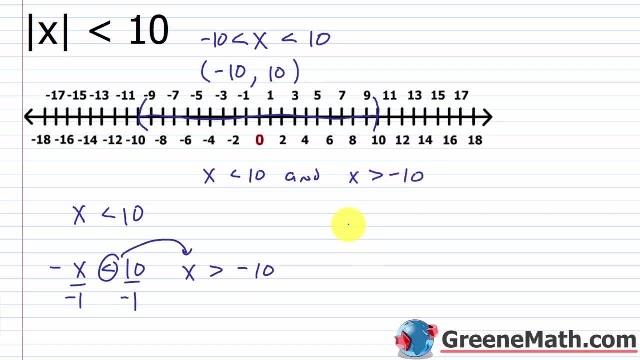 and x is greater than negative ten, which we write as a three part: x is greater than negative ten and x is less than ten. so that's where all this comes from. so now let's look at one that's a little bit more challenging. this is something you'll see at the very 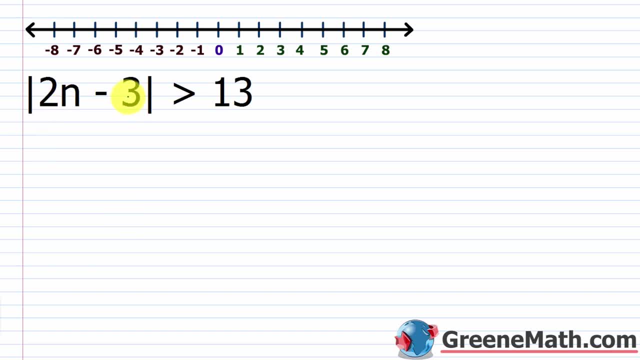 very first part. so we have the absolute value of two n minus three is greater than thirteen. so the first thing to make sure of is that the absolute value operation is isolated. so this is isolated. you have an inequality symbol and then some number. now the next thing you think about is: is it a? 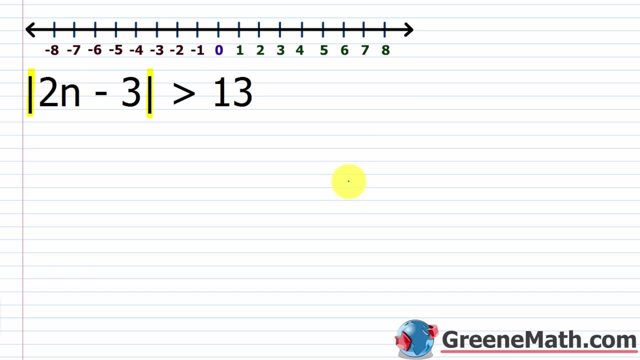 greater than, or is it a less than? in this case it's a greater than so, with a greater than we have. or we set up a compound inequality with or so. the first one is: remove the bars, so two n minus three is greater than thirteen. then, or the second. 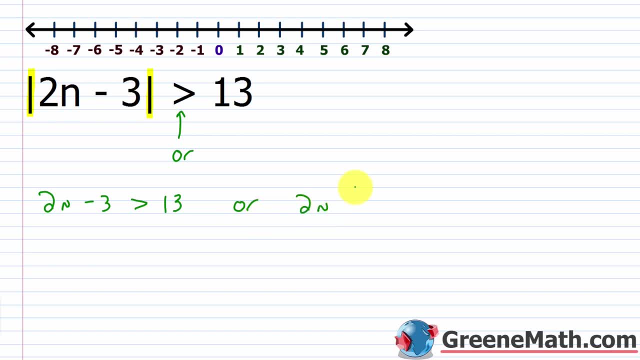 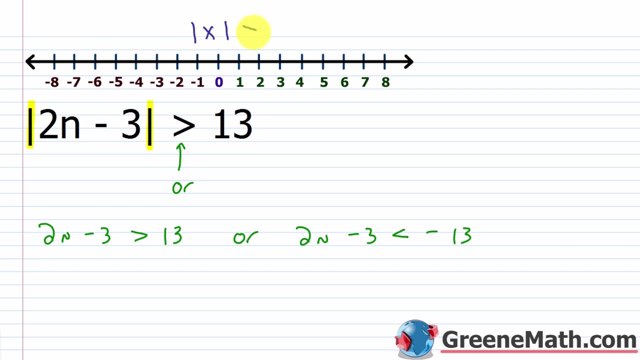 one is: remove the bars, so two n minus three. flip the sign so it's a less than make this negative, so negative. thirteen again: the easy way to remember this: go back to your generic example. the absolute value of x is greater than k, so this turns into: 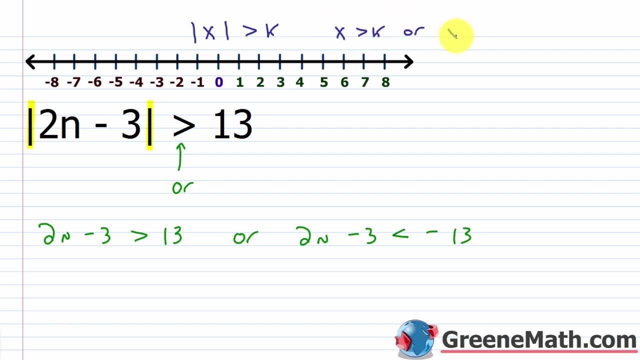 x is greater than k or x is less than negative k. just use this as an example on the first few and you'll remember. the first one is: just remove the bars as we have here. just remove the bars we have. x is greater than k. the second one is: 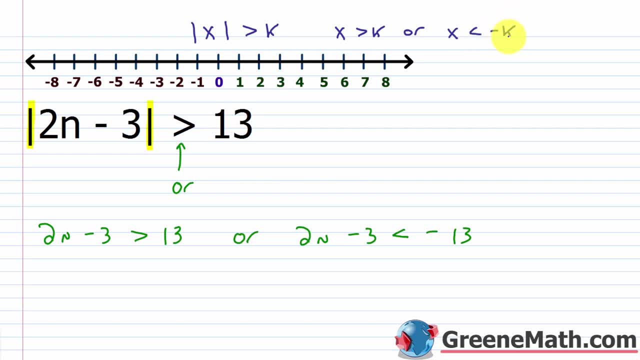 remove the bars, flip the sign, make it negative. so we remove the bars, we flip the sign from greater than to less than. we made thirteen, negative thirteen. and again where this comes from, if i took the negative of this, so let's say i have the negative of this whole expression. 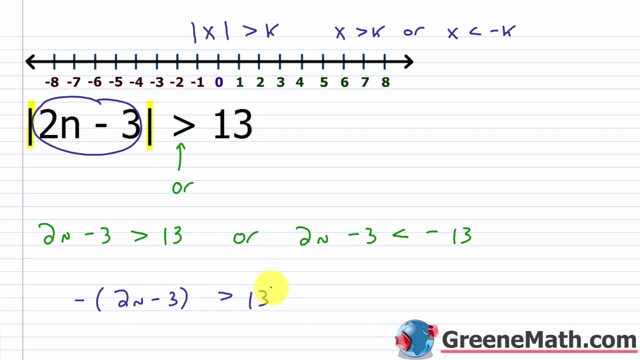 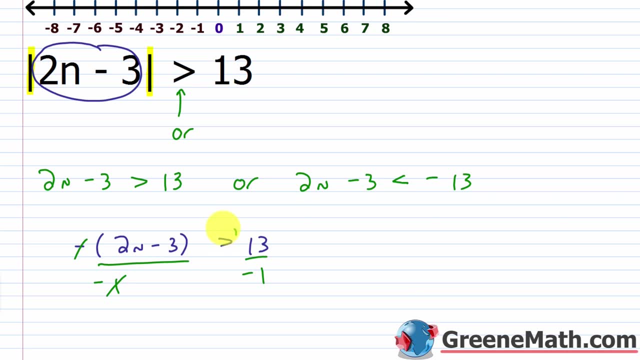 two n minus three is greater than thirteen. what i can do is divide each side by negative one, and i can cancel this. divide this by negative one, but this gets flipped. so you get two n minus three, which is this: flip the sign. okay, that's why we 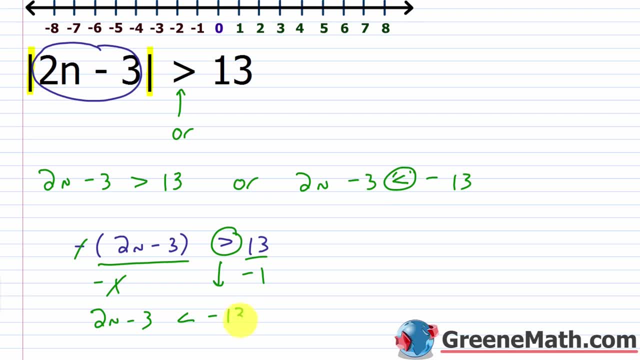 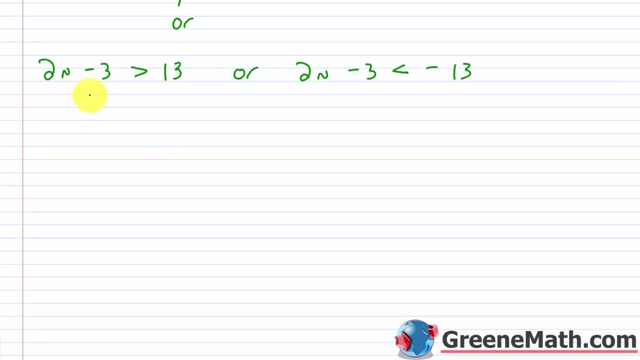 flip here and then we make this negative. so this is negative thirteen. so again, that's where this is coming from. alright, so let's erase everything. let's get our solution. let's scroll down a little bit. so i just want to solve this like i normally would. so i'd 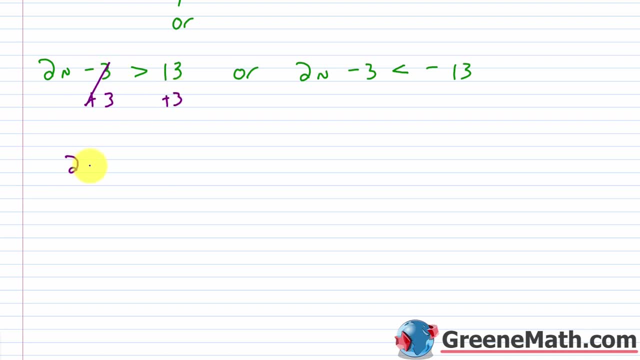 add three to each side here. that will cancel two n is greater than sixteen. divide both sides by two and i get n is greater than eight over here. i'll add three to each side. that'll cancel, and i'll have two. n is less than negative. thirteen plus three is negative. 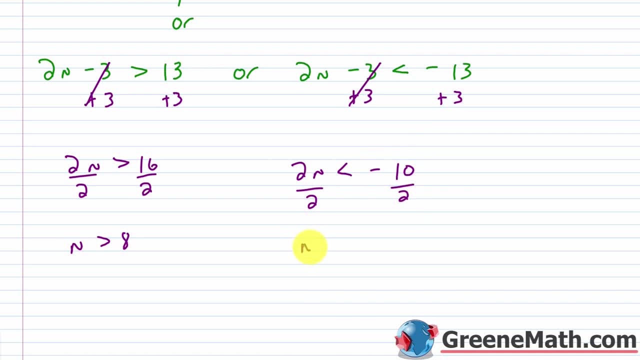 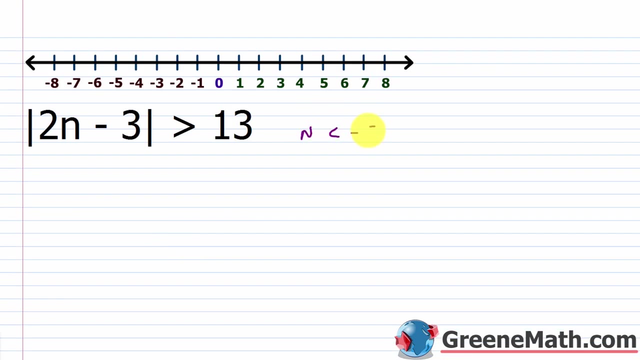 ten. divide each side by two and we'll get that n is less than negative five. so i get n is greater than eight or n is less than negative five. so let's go back up and notate this. so your solution here would be again: n is less than negative five. 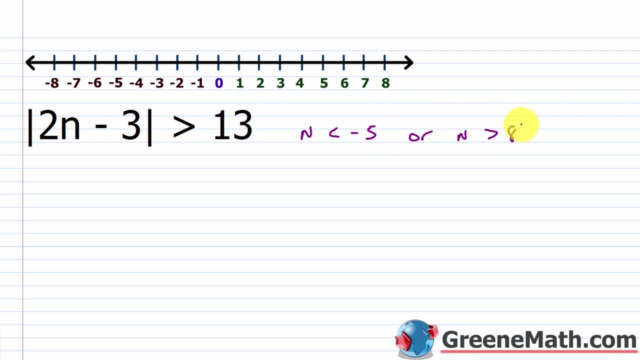 or n is greater than eight. in interval notation i could write from negative infinity up to, but not including negative five, and it's the union with this other set which is anything larger than eight out to infinity. now, graphically, at negative five, i'd put a parenthesis facing to the left. 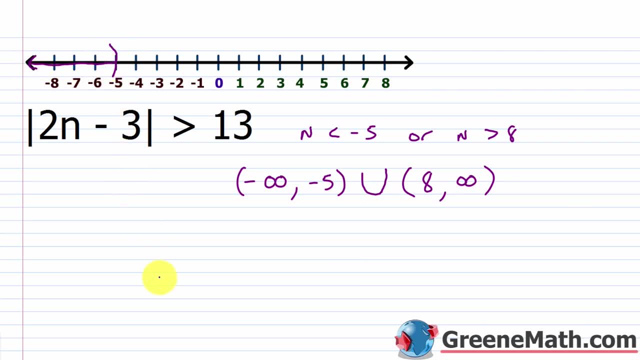 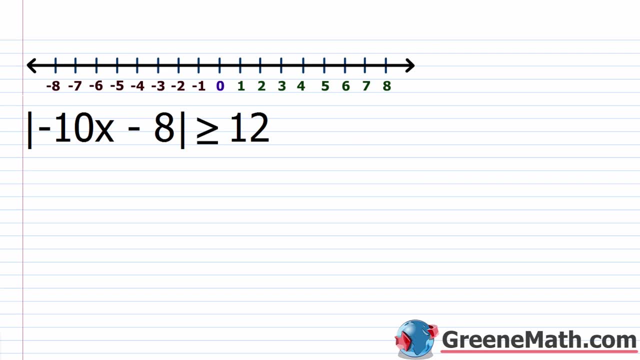 and i'd shade everything this way. and at eight i'd put a parenthesis facing to the right and i'd shade everything this way. alright, let's take a look at another one. so we have the absolute value of negative. ten x minus eight is greater than or equal to twelve. 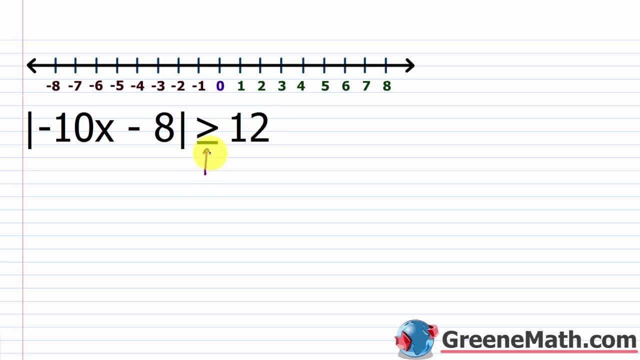 so again i'm looking at a situation with a greater than. doesn't matter that it's a greater than or equal to, it's just going to change the notation a little bit. if i have a greater than involved, or greater than or equal to, it's a. 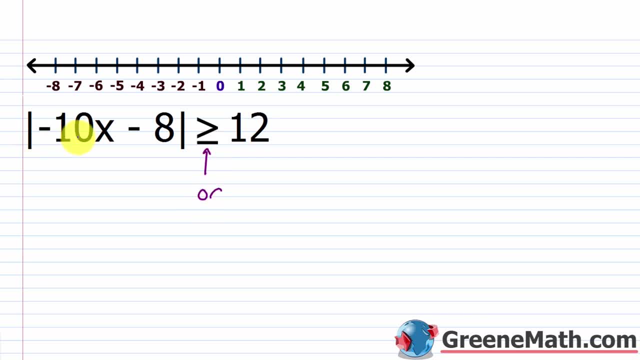 compound inequality with: or so i remove the absolute value bars. so negative ten x minus eight is greater than or equal to twelve. then or remove the absolute value bars. negative ten x minus eight. flip the sign. so now this is a less than or equal to make this negative, so negative twelve. 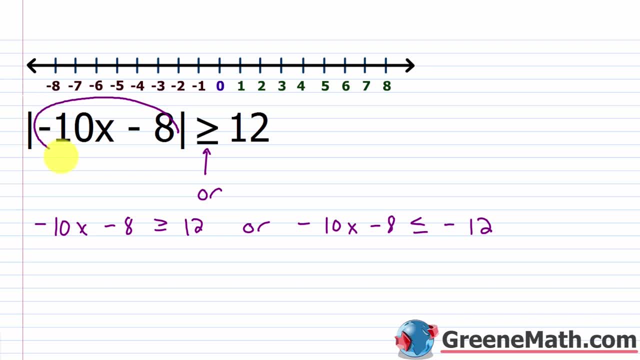 and again that comes from the fact that i can have the negative of this be greater than or equal to twelve. i divide both sides by negative one. this becomes negative and the sign gets flipped. it's just that simple. so let's go ahead and solve each one here. 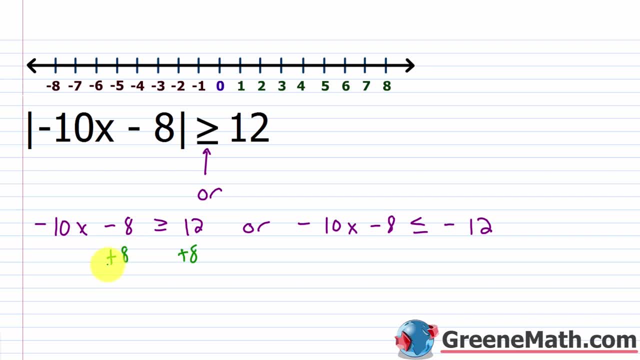 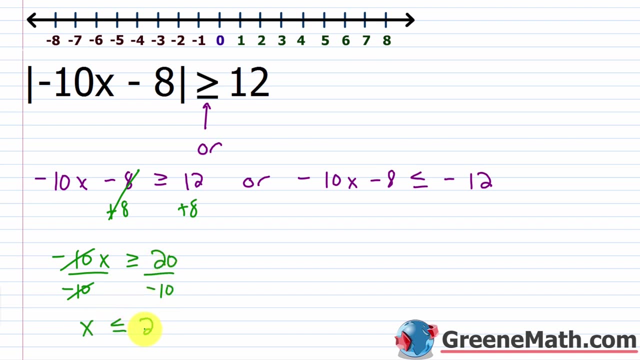 so we'll have plus eight and plus eight. that cancels negative ten. x is greater than or equal to twelve. plus eight is twenty. divide both sides by negative ten and this will cancel of x is less than or equal to twenty. divided by negative ten is negative. 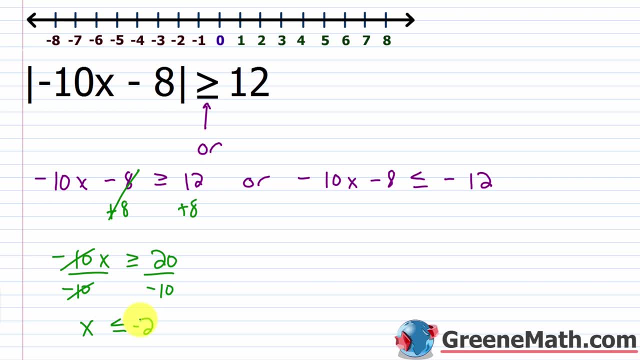 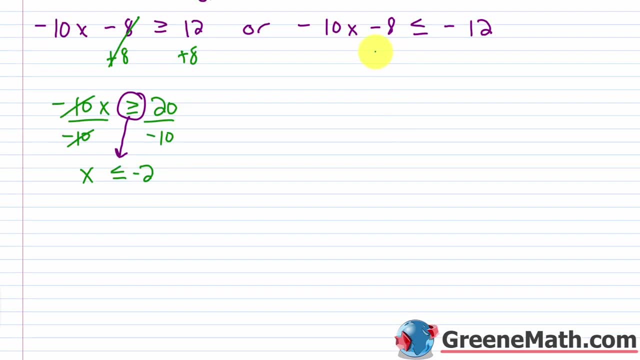 two. so x is less than or equal to negative two. and again, because i divided by a negative, i flipped the direction of that inequality symbol. okay, for this side. i'm going to add eight to each side to begin. that'll cancel. i'll have negative ten x. 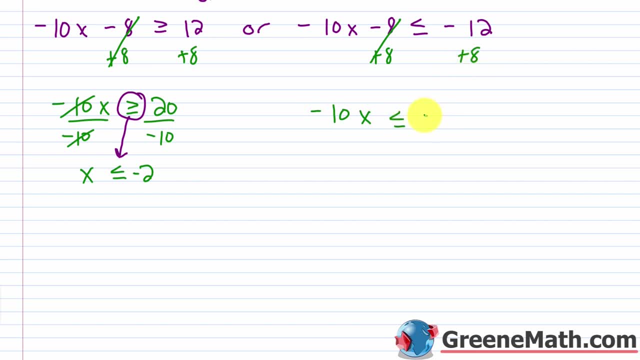 is less than or equal to negative. twelve plus eight is negative four. let's go ahead and divide both sides by negative ten, and if i divide by a negative i flip the direction of that inequality symbol. so this is going to be a greater than or equal to. 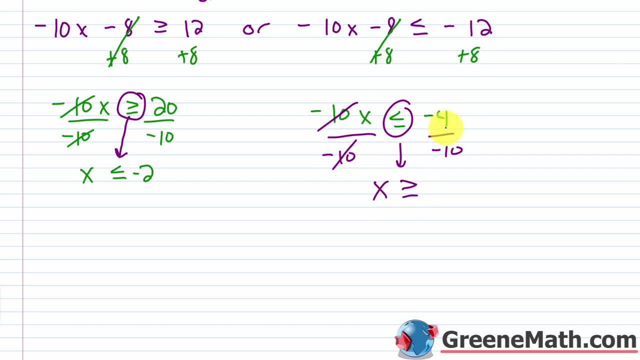 now this cancels. x is greater than or equal to negative four over negative ten. i know that negatives would cancel, so this would be positive. each is divisible by two. four divided by two is two. ten divided by two is five. so x is greater than or equal to two-fifths. 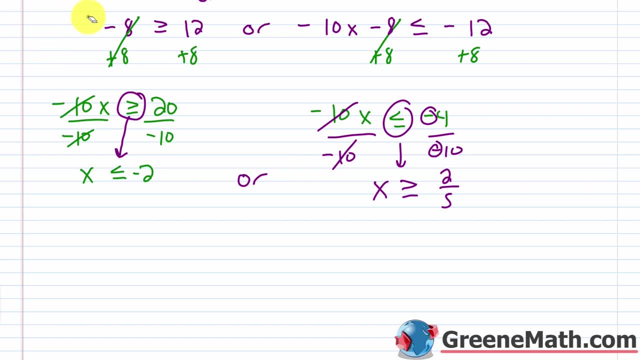 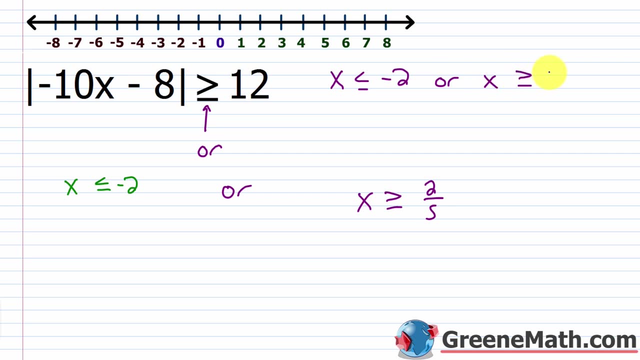 there. so this is an or, and let's erase everything and notate this properly. so we have: x is less than or equal to negative two, or x is greater than or equal to two-fifths. in interval notation again, it's the union of the two solution sets. so 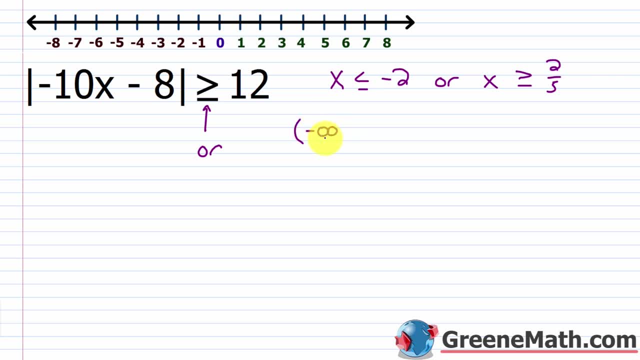 it's anything. we have negative infinity out here, as the smallest up to and including negative two. so i'm going to use a bracket and then the union with this guy, so including two-fifths and anything larger. so graphically i can find negative two on the. 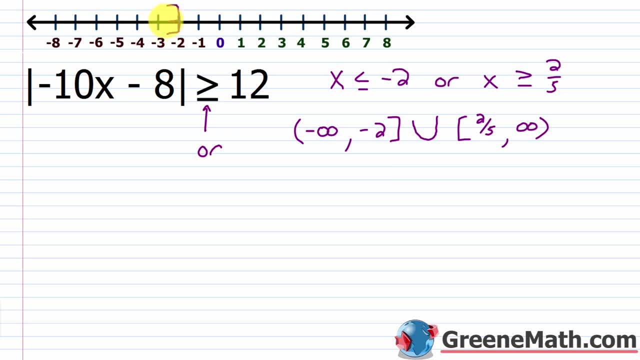 number line that's here, put a bracket facing to the left and shade everything going this way. now two-fifths doesn't have a notch, but two-fifths is point four as a decimal, so it's a little bit less than a half, so let's just say it's like: right there. 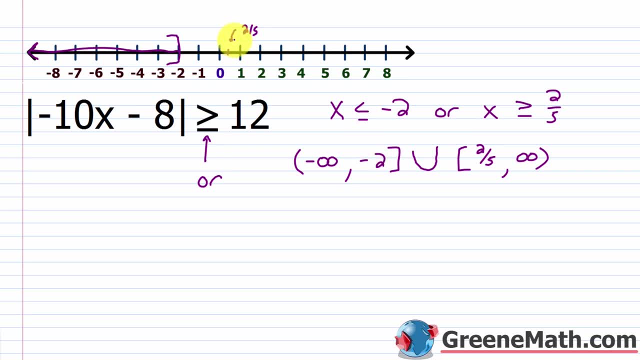 let's say this is two-fifths, and again it's anything that includes two-fifths, so that value or larger. and again, if you have this on a test, your teacher is going to allow you to make notches where they're on right. they understand that, so it's. 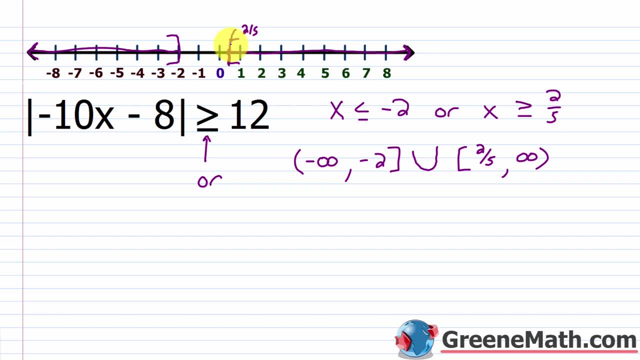 not perfectly at two-fifths, but you know, you've notated where it is. that's the best you're going to be able to do so again. anything that is less than or equal to negative two, along with anything that is two-fifths or greater, would be a solution. 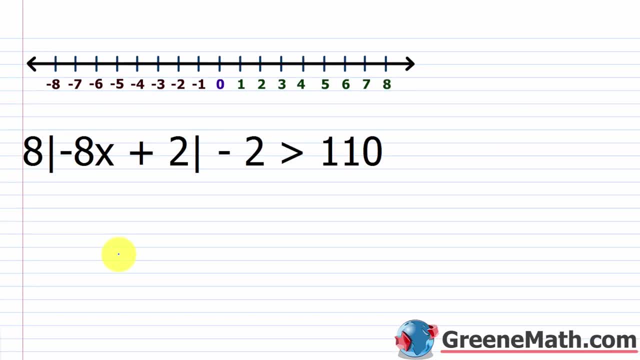 for this inequality. alright, let's take a look at another one. so we have eight times the absolute value of negative. eight x plus two minus two is greater than a hundred ten. so common mistake is: after you've seen these easy problems, you go through and you start. 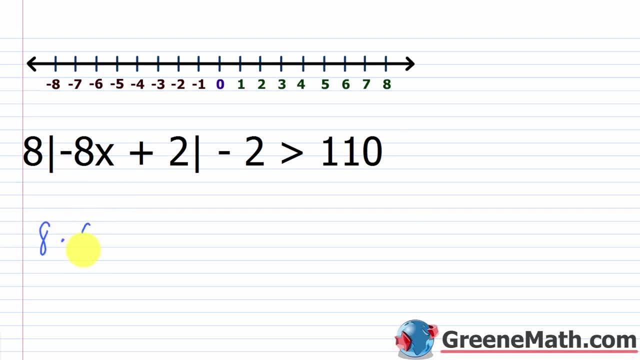 saying okay, well, eight times. remove the bars. negative eight x plus two minus two is greater than a hundred ten. or then you take this and you say: well, eight times, and then, inside parentheses: negative eight x plus two minus two is less than negative a hundred ten. no, 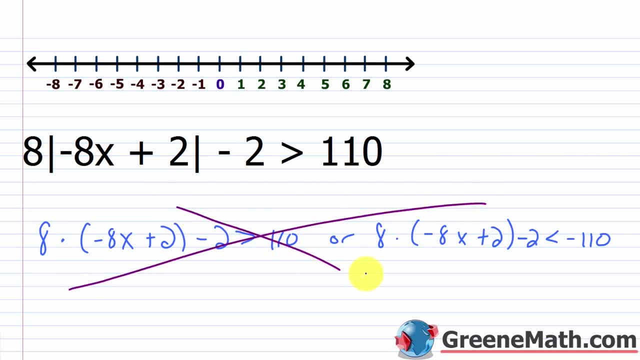 okay, do not do this wrong. you have to isolate the absolute value operation first. you want it to look like this: the absolute value of something- let's just say x, doesn't matter what it is- is greater than some value k. so this x could be anything, could be the absolute value of. 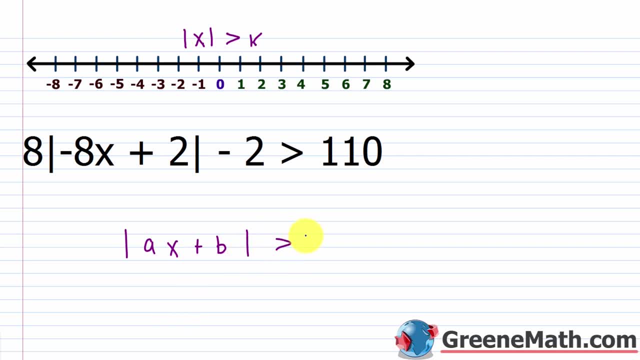 ax plus b- if you want to make it more complicated- is greater than k. this leads to what x is greater than k or x is less than negative k. this, the more complicated example, just leads to: ax plus b is greater than k or ax plus b is less than negative. 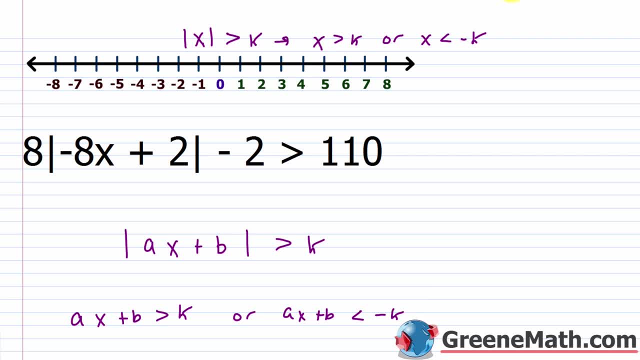 k. okay, so the main thing here is to isolate the absolute value operation first, and then just follow this formula here, write it on a flash card and keep using it. alright, let me erase this real fast and let's go ahead and simplify. so I'm going to add two. 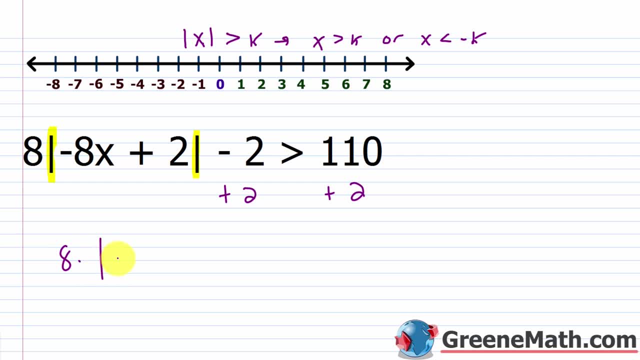 to each side, I'll have eight times the absolute value of negative. eight x plus two. this is greater than a hundred. ten plus two is a hundred twelve. now I want this by itself. I have multiplication here, so I'm going to use division to get it by itself. 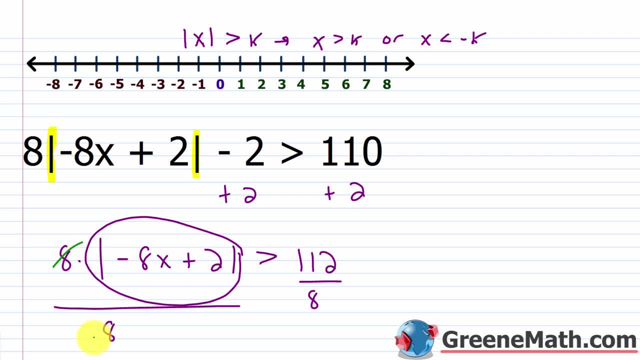 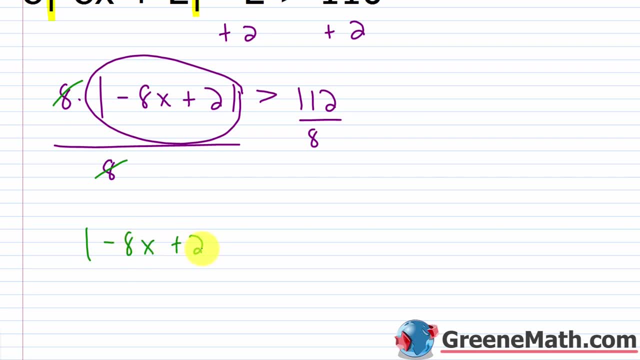 divide both sides by eight, and so this will cancel. with this, just scroll down and get some room going and I'll be left with the absolute value of negative. eight x plus two is greater than what's a hundred twelve divided by eight. well, most of us don't know that off the top of our heads, but punch it. 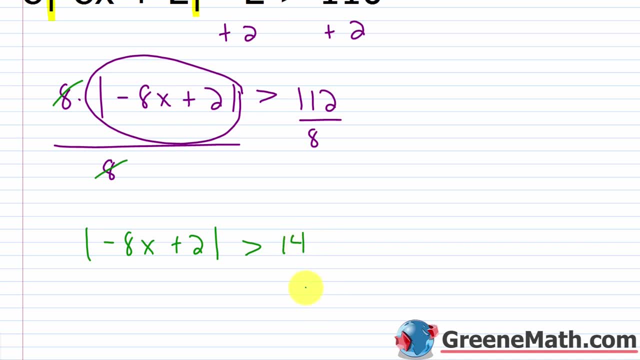 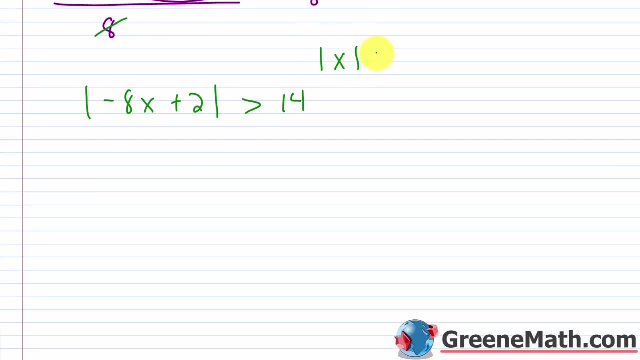 up on a calculator and you'll get fourteen. now I have something that is matching again what I saw earlier: the absolute value of something, let's just say x, is greater than k, so the absolute value of negative eight x plus two is greater than fourteen. remember this: sets. 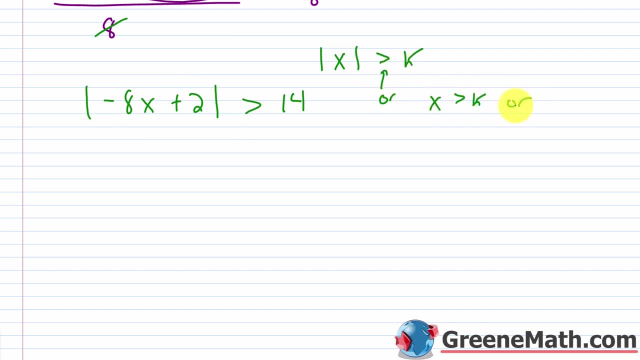 up as: or so x is greater than k or x is less than negative k. same thing. this is, or so we have negative eight x plus two is greater than fourteen. all I did was just remove the absolute value bars then. or remove the absolute value bars, so negative eight x. 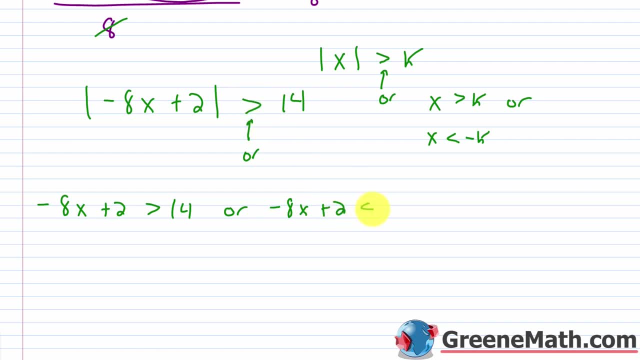 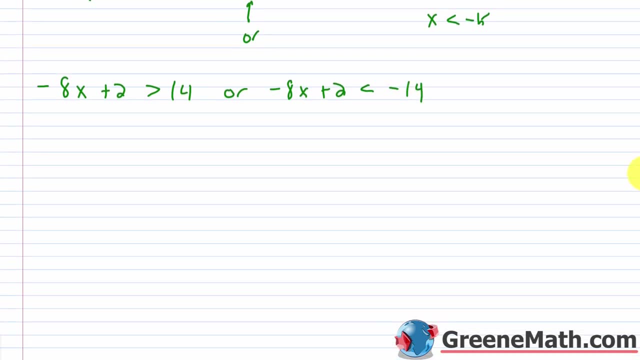 plus two flip this direction here. so this is a less than make this negative negative fourteen. so you're basically good to go at this point. you just need to find your solution for this. so we're going to subtract two away from each side and that'll cancel. 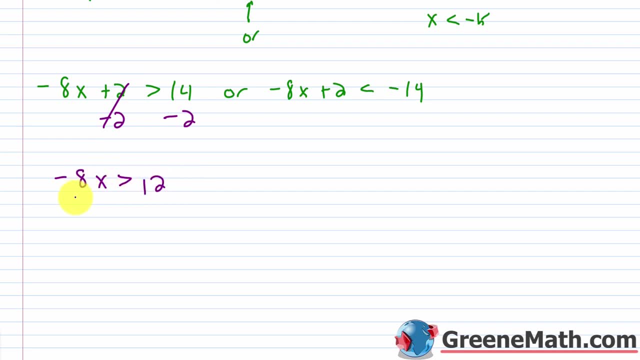 I'll have negative eight. x is greater than twelve. divide both sides by negative eight. you're going to flip the direction of this guy. this will be a less than this cancels with this. I'll have: x is less than twelve over negative eight. each is divisible by two. 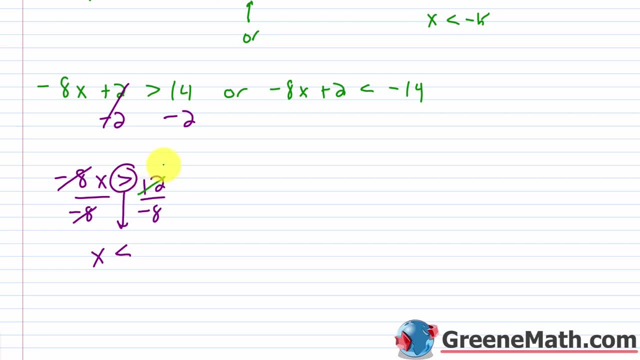 in fact each is divisible by four. so if I divide this by four, I get three. if I divide this by four, I get negative two. so let's put negative three halves and then let's look at the other guy. so if I subtract two away from each side, 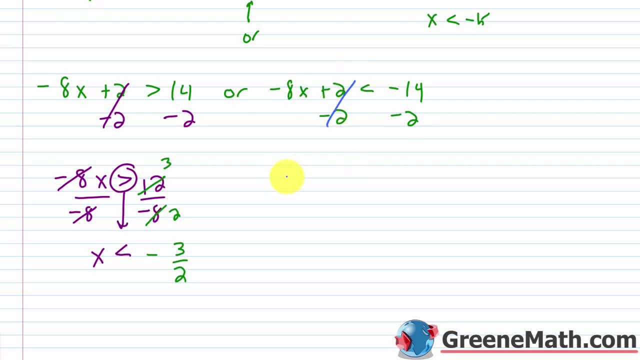 over here. this is going to cancel. I will have negative eight. x is less than negative. fourteen minus two is negative sixteen. divide both sides by negative eight, so this will cancel with this and what I'll have is x and I've got to flip. this is greater than. 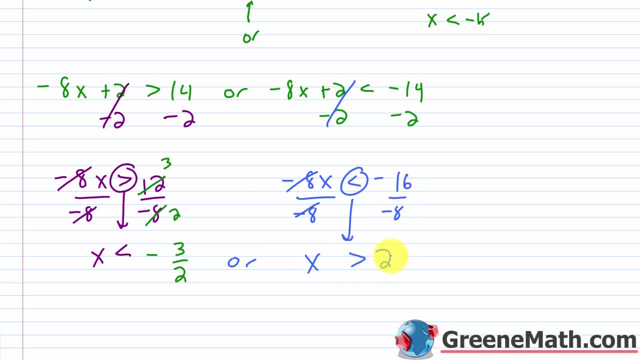 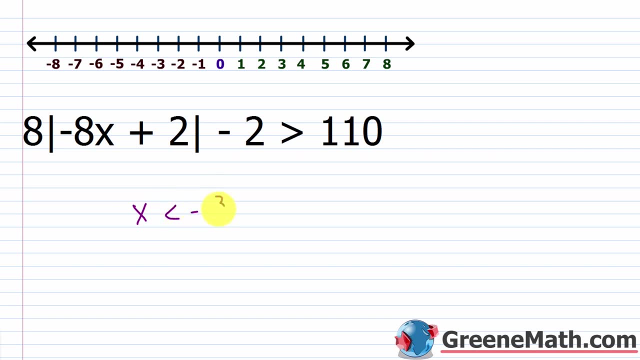 negative sixteen over negative eight is two. so x is less than negative three halves or x is greater than two. so again we found that x was less than negative three halves or x was greater than two. so in interval notation it's the union of the two solution. 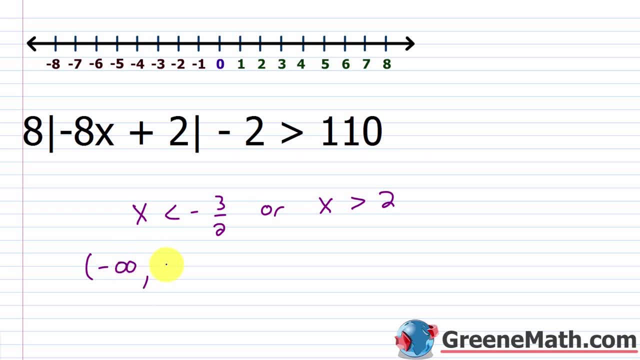 sets. so coming from negative infinity up to, but not including negative three halves and the union with this other guy after two right anything larger, out to infinity, graphically I don't have a negative three halves, but negative three halves is negative one point five. so it's between negative 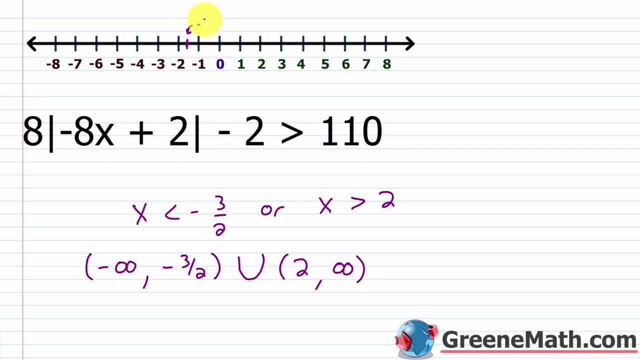 one and negative two. so let's just say it's right there. this is negative three halves. it would be anything less than that, so I'll put a parenthesis facing left, shade everything to the left and then anything larger than two. so put a parenthesis at two and we'll shade everything to the. 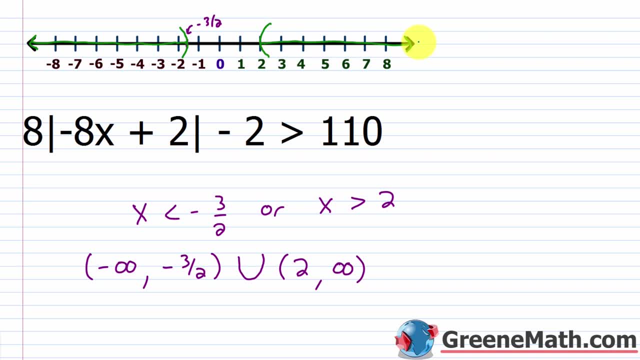 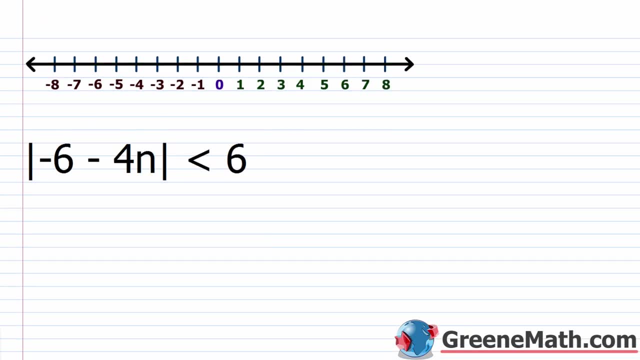 right. so again, x can take on any value that is less than negative three halves, or it can also take on any value that is larger than two. alright, let's take a look at one now, where we have a less than so, we have the absolute value of negative six minus. 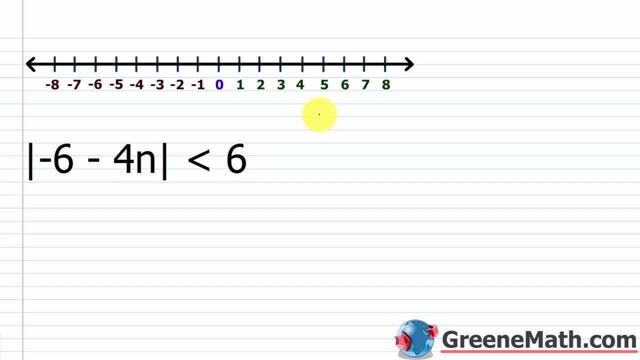 four, n is less than six. so again, if we see something in this format, the absolute value of x is less than k. it's a compound inequality with and, so x is less than k, but it's also greater than the negative of k. ok, so you have, x is less than. 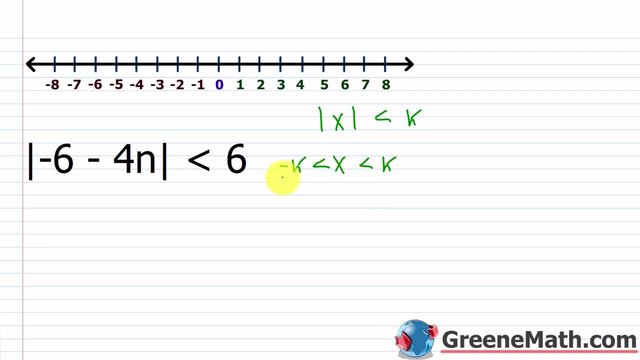 k and x is greater than the negative of k. so I'm going to take this part right here and I'm going to say: negative six minus four, n is less than six. so the same as it looks right here. just drop the absolute value bars then and ok, now you have. 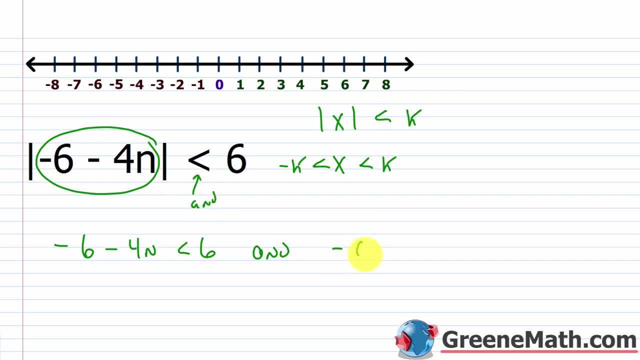 and because you have a less than, it's also true that negative six minus four n is greater than. flip the sign just like you do before. make this negative, so negative six. so negative six minus four n is greater than negative six. so we can write this as a three part inequality. make it. 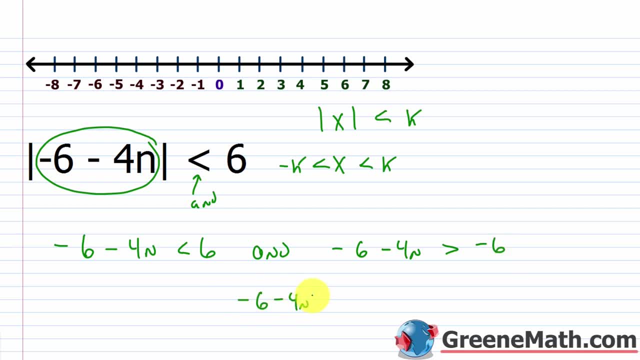 easy on ourselves. so we have negative six minus four n in the middle. it's greater than negative six and it's less than positive six. so I can just erase this and I can drag this up here and again. if you're wondering where this came from, I've showed it multiple times, but 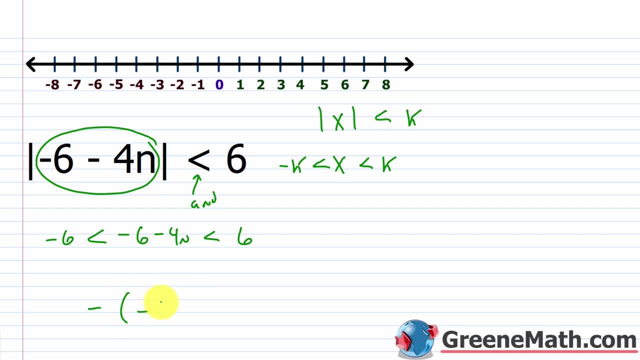 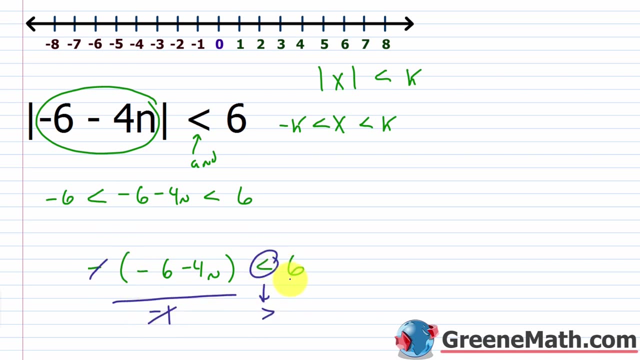 it's basically that we take the negative of this, so negative of negative six minus four n, this is less than six because of the absolute value operation. that would work as well. and then we divide both sides by negative one, so this cancels. that makes me flip the sign. and then 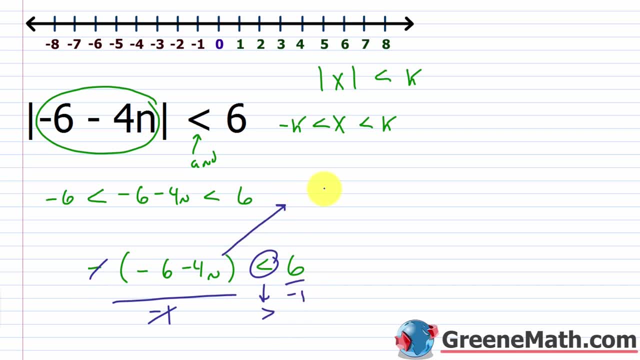 this becomes negative six. so we have this guy right here, negative six minus four n the sign is flipped and then we have negative six. so that's where this part right here comes in. let me erase all this now and let's just attack the problem. so if I 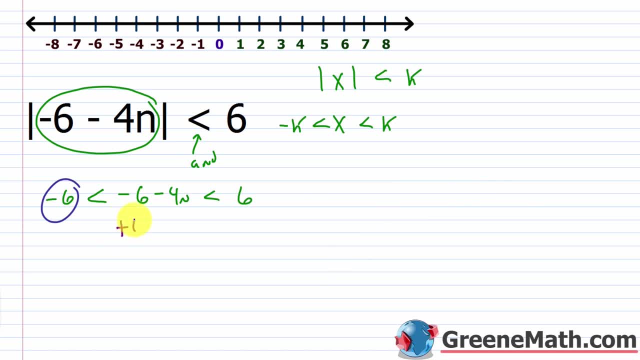 solve this three part inequality. I do the same thing to each part. I'll add six over here and over here, so that'll cancel becomes zero. that'll cancel. I'll have negative four. n is less than six plus six is twelve. so I divide each part by negative four. 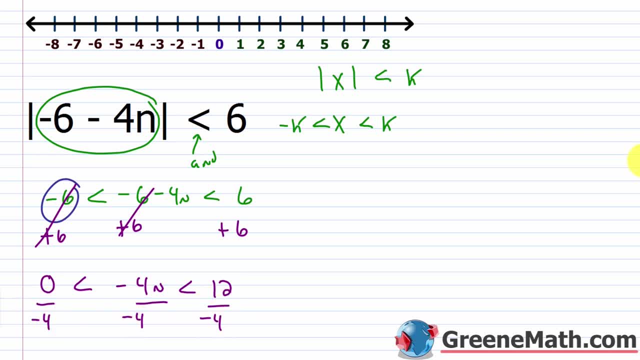 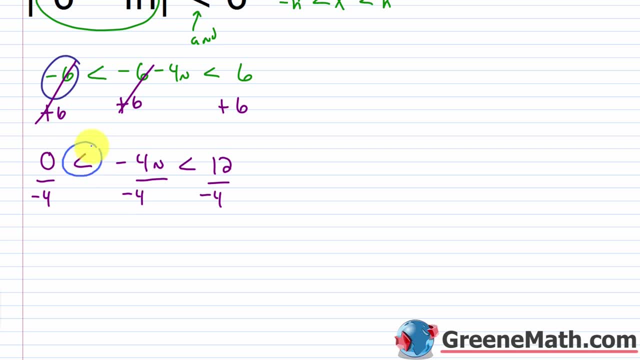 so I can isolate n and what's gonna happen is, again I've got to still flip the direction. when I have a three part inequality and a divide by a negative, that doesn't change. so this gets flipped and this gets flipped. so this is greater than this is greater than this cancels with this. 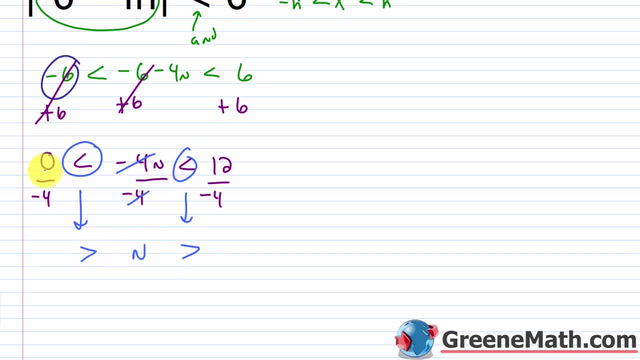 and I'll have n. so n is less than zero. divided by negative four is zero and it's greater than twelve. divided by negative four is negative three. so generally we don't leave it in this manner. we rearrange it to where it's, in the direction of the. 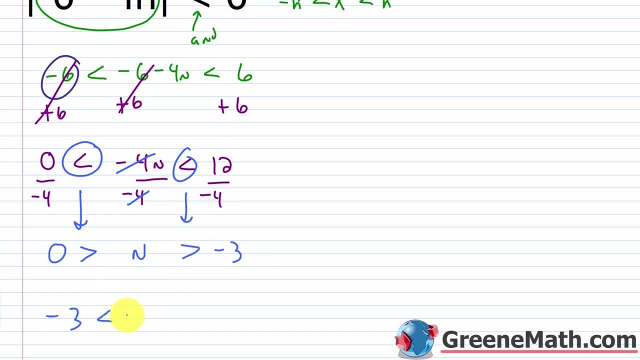 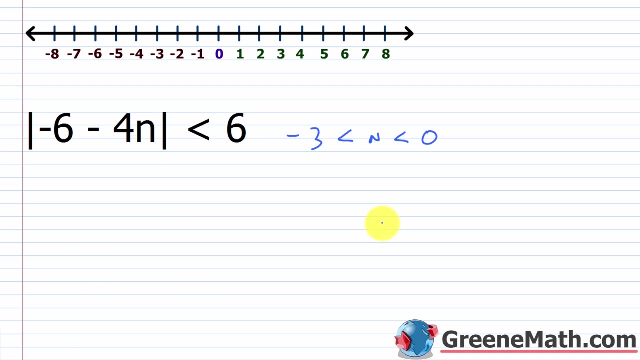 number line. so negative three would be here. of course that's less than n and we know that n is less than zero. so let's take this solution up and we're gonna graph it and use it to write an interval. so n is greater than negative three and less than zero. 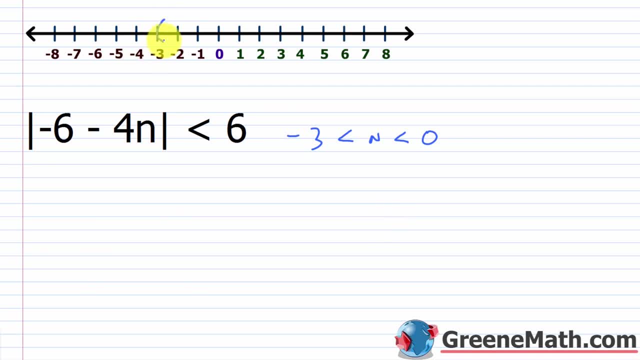 so here's negative three, so it's greater than that and it's less than zero. so it's between negative three and zero. so that's what it looks like graphically in an interval notation. I just have the interval greater than negative three but less than zero. 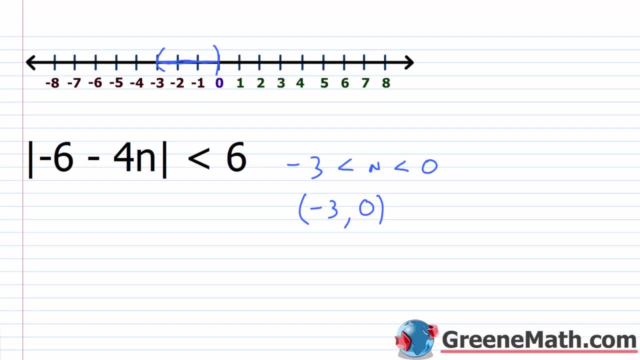 just like that. so n again can take on any value that's greater than three but less than zero. alright, for the next one. we're looking at seven times. the absolute value of ten k plus three plus seven is less than twenty eight. so again I want to isolate the absolute. 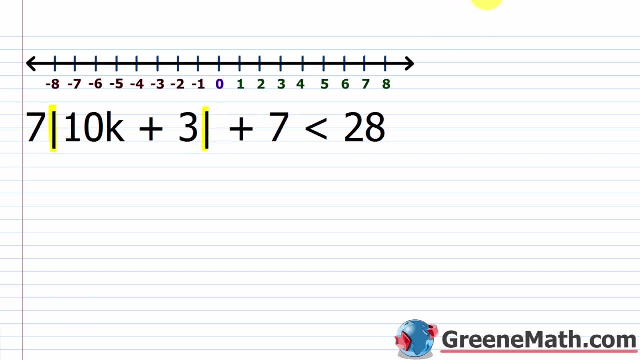 value operation. before I do anything, don't make the mistake of just trying to apply the rule before you have isolated the absolute value operation. so I want to subtract seven away from each side first. I'll have seven times the absolute value of ten k plus three. this is less than. 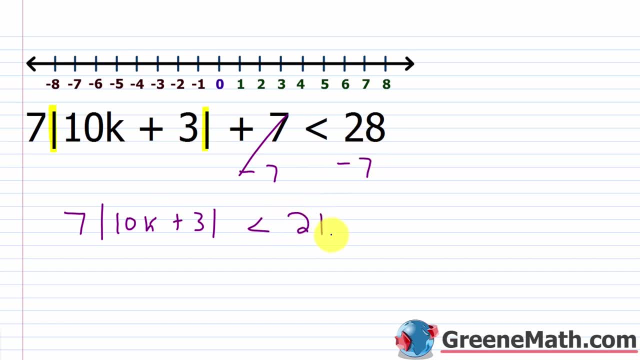 twenty eight minus seven is twenty one. so now I can divide both sides by seven, and when I do that this will cancel. with this I've isolated my absolute value operation. it's the absolute value of ten k plus three, and this is going to be less than twenty one divided by seven. 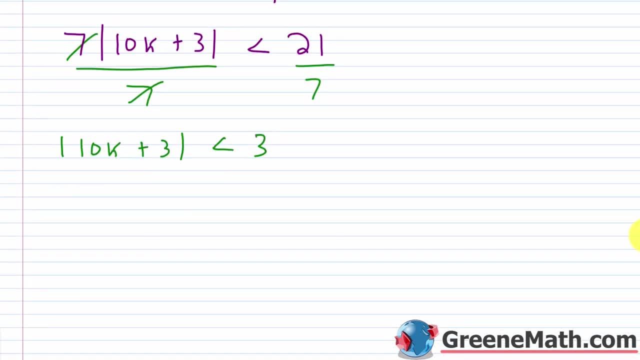 is three. so now I can go ahead and apply my little formula: remove the absolute value bars, so I'll have ten k plus three, and then it's just less than three, and the other scenario would be that ten k plus three. remove the absolute value bars, flip the direction. 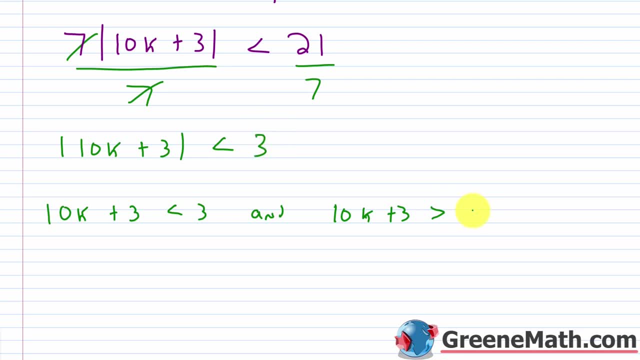 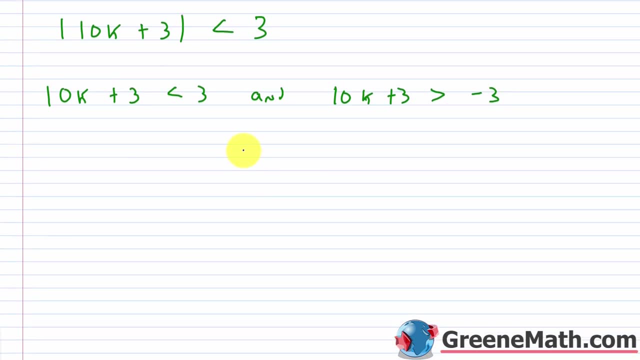 of the inequality symbol, so it's greater than, and then make three negative, so negative three. and again, to make this easier on yourself, write it as a three part inequality. so go ahead and write this as ten k plus three is greater than negative three and less than three. 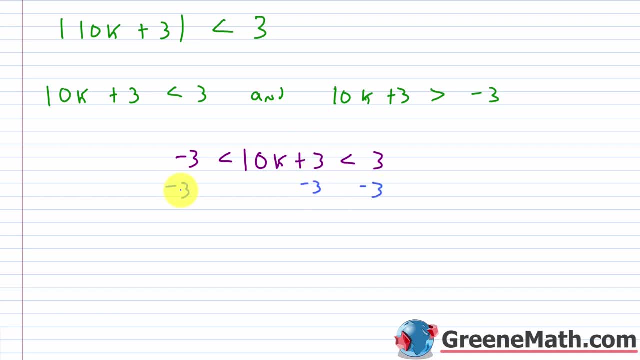 so let's subtract three from each side, so this will cancel negative. three minus three is negative six. this is less than we'll just have ten k now, and it's less than three minus three is zero. divide each side by ten. this will cancel with this and I'll have k in the middle. 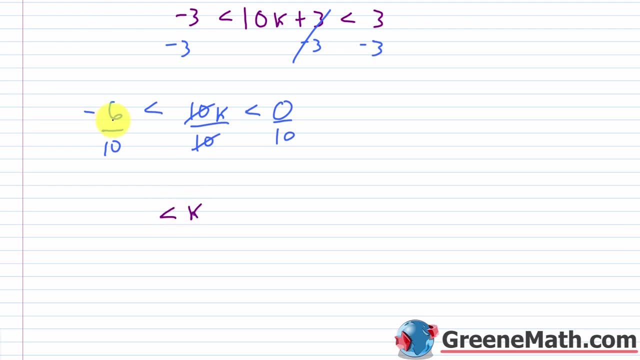 by itself, which is what I want, and it's going to be greater than negative six over ten. I know it's negative six is divisible by two. six divided by two is three. ten divided by two is five, so negative three fifths and zero divided by ten is, of course, 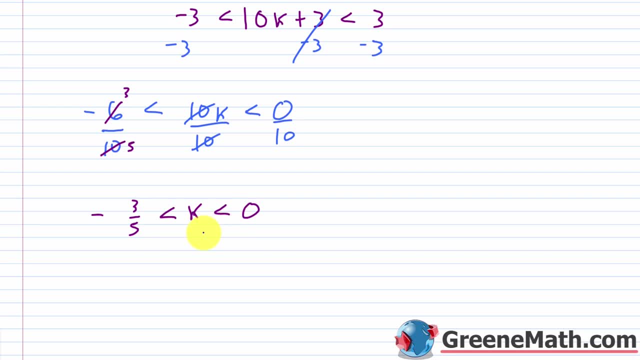 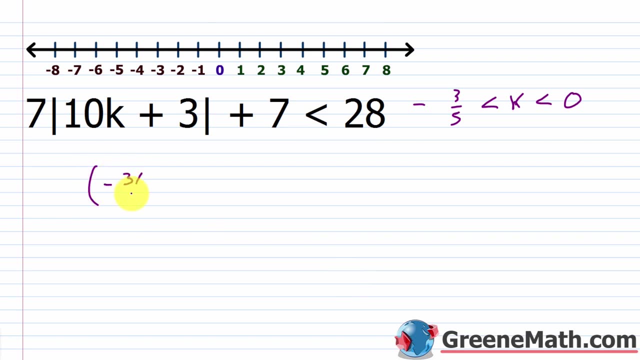 zero. so then less than zero. so k is greater than negative three fifths and less than zero. so in interval notation that's not including negative three fifths up to, but not including zero. so let's look at that and then on a number line, where is negative three fifths? 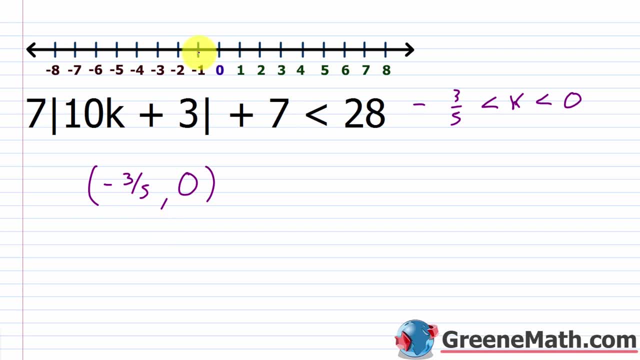 well, it's negative point six. so if you look between zero and negative one, it'd be a little bit past negative point five. so let's say, about right there, we could say this is negative three fifths. so here's zero. so what I would do is I would put. 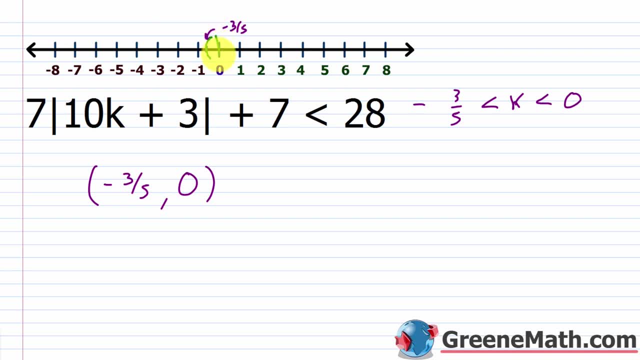 a parenthesis here facing to the right one, here facing to the left. it's kind of a small area on our number line we'd shade everything in between. so again, k can be anything that is greater than negative, three fifths up to, and not including zero. so 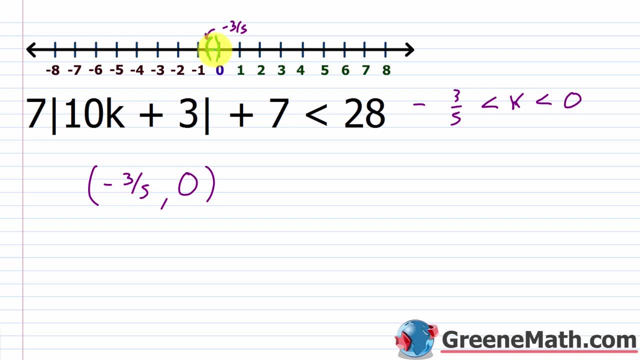 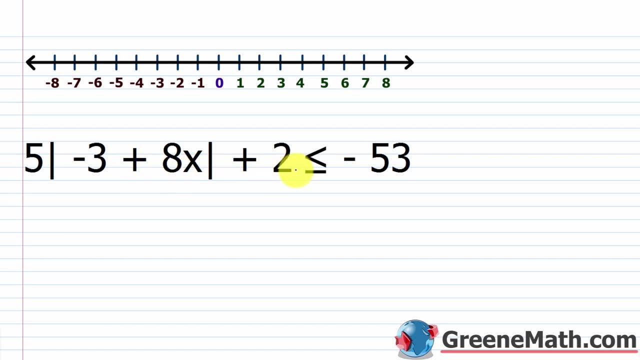 anything in that range between, again, negative three fifths and zero. for the last problem we're going to look at, we have five times the absolute value of negative three plus eight. x plus two is less than or equal to negative fifty three. so again I want to isolate the absolute value operation. 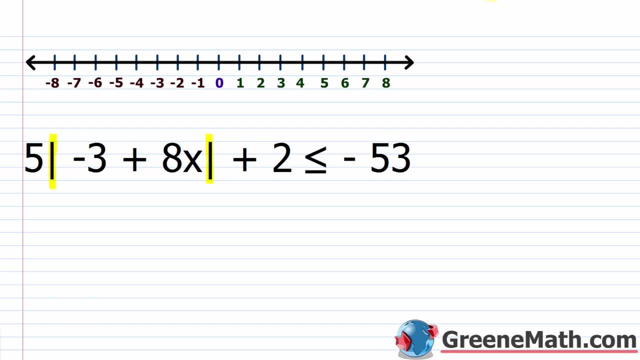 first, don't just start applying rules to stuff. that's a common mistake. so let me subtract two away from each side of the inequality. that'll cancel. I'll have five times the absolute value of negative. three plus eight x, and this is less than or equal to negative fifty three. 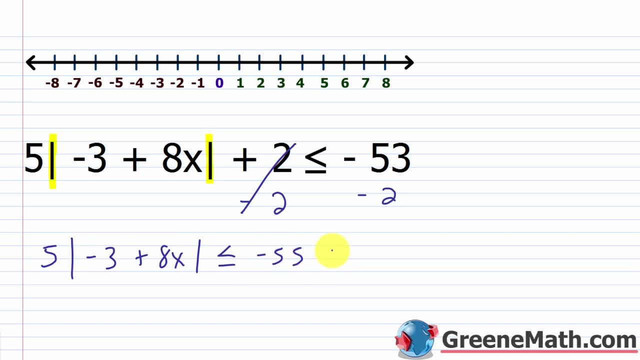 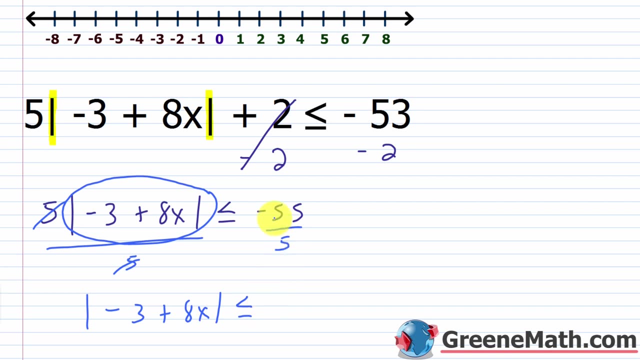 minus two is negative fifty five. so now let me divide both sides of the inequality by five, so again I can isolate this part right here. this'll cancel with this and I'll have the absolute value of negative. three plus eight x is less than or equal to negative. 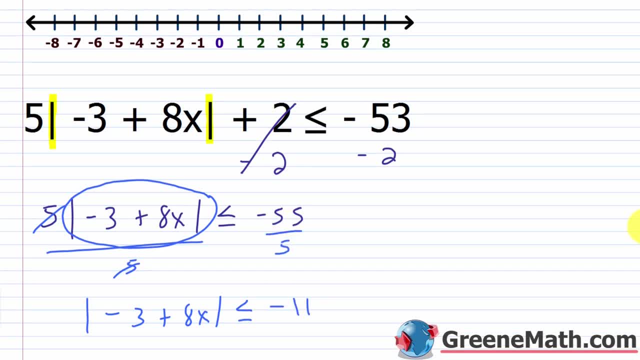 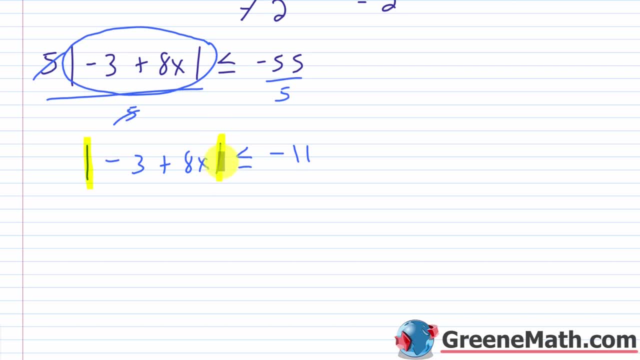 fifty five over five is negative eleven. now am I going to continue with this? no, I am not. why think about this? the absolute value operation produces a result that is zero or it is positive. it cannot ever be less than or equal to negative eleven. that's not going to work. it can't be. 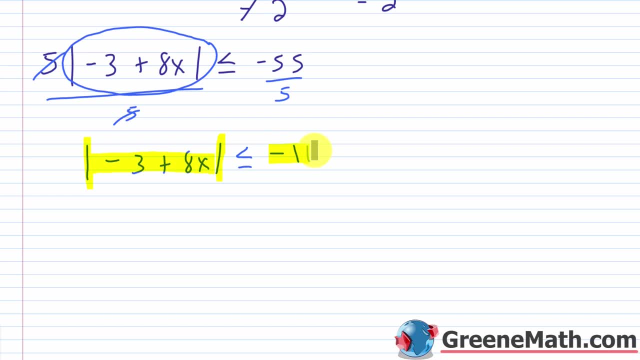 less than a negative value. it has to be greater than or equal to zero. so this has no solution. this has no solution. and again, when you see something with no solution, you can say the solution set has no elements. so you put the symbol for the null or empty. 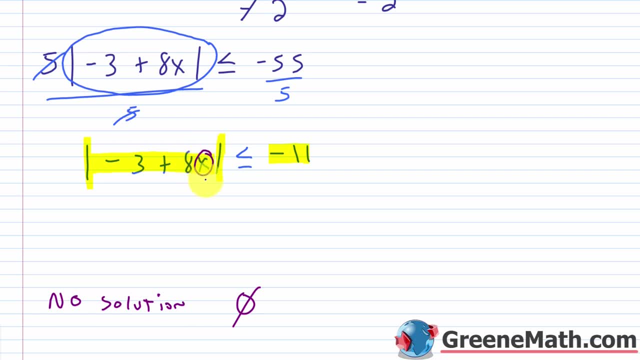 set one more time. if I try to plug in something for x, multiply by eight and add negative three, when I take the absolute value of it, the absolute value will never be less than or equal to negative eleven. it won't ever happen because the absolute value is either zero. 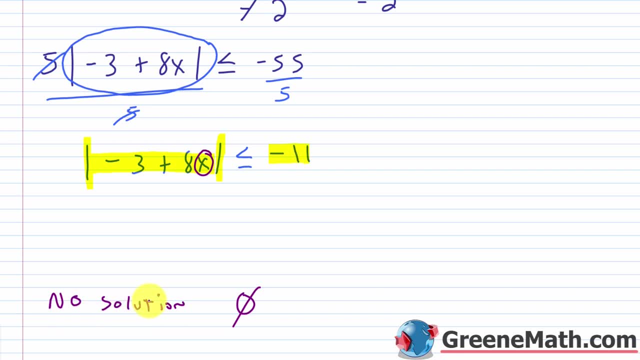 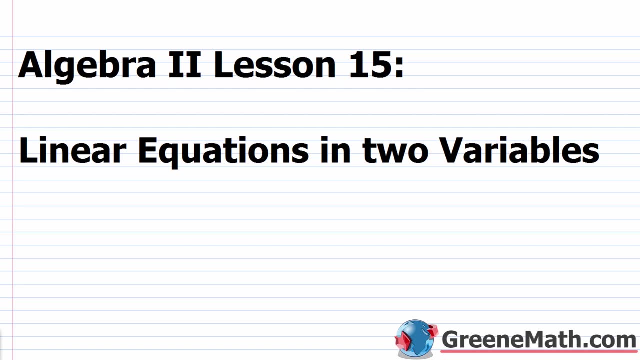 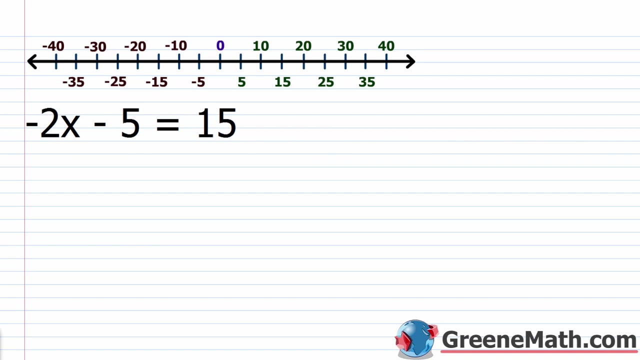 or it's positive. so that's why, again, there's no solution. hello and welcome to algebra two, lesson fifteen. in this video, we're going to learn about linear equations in two variables, so this is not a new topic for us. in algebra two, we learned about linear equations in two variables in 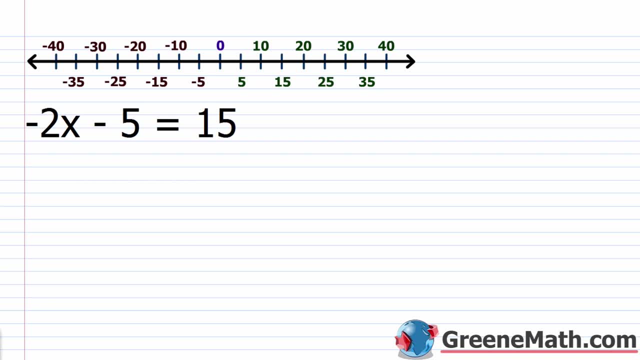 algebra one. but for some of you you never took an algebra one course, and for others you kind of stumbled through your algebra one course. so it's important to get a good full review here. so the first thing I'm going to talk about is up to this point. 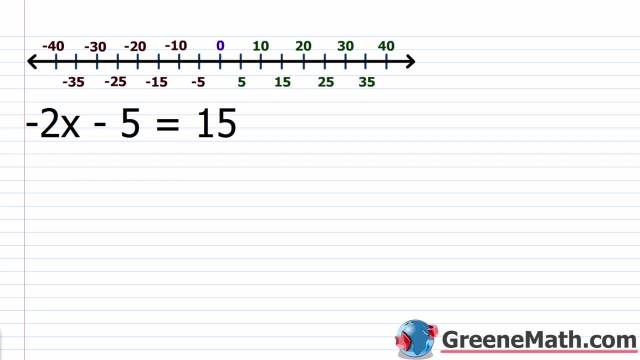 we've only kind of worked with a linear equation in one variable. we also talked about linear inequalities in one variable and some variations on that. we looked at some absolute value stuff and some compound stuff, you know so on and so forth. but the main idea here is that a linear equation 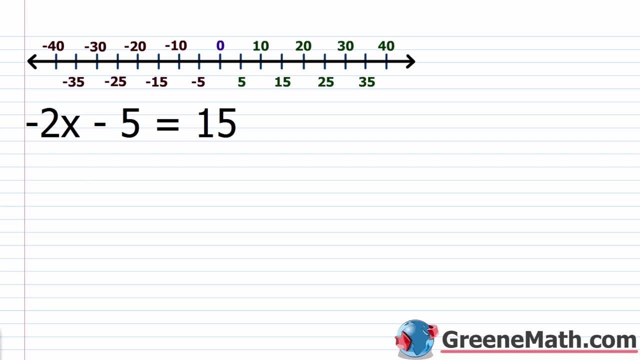 in one variable has generally one and only one solution. so for this type of problem, let's say I have negative two x minus five equals fifteen. I add five to each side of the equation. I have negative two x is equal to twenty. I divide both sides by: 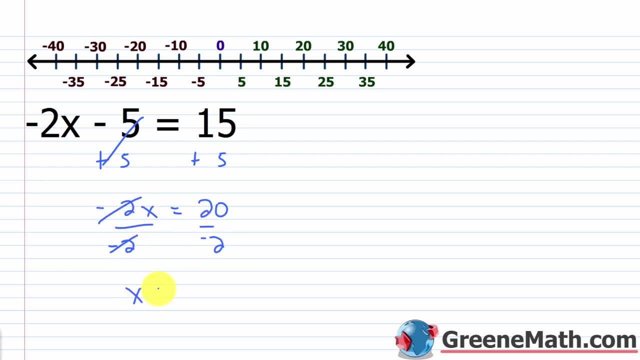 negative two and I get a single number. I get that x is equal to negative ten. so using a number line, I can display that visually by saying: this is my solution for this equation: negative two x minus five equals fifteen, and again that means that if I replace x with 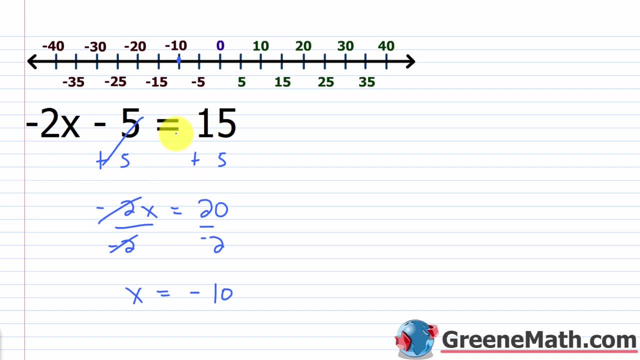 negative ten, I would get the same value on the left as I have on the right. so that at this point we should all know- and let me go ahead and write that in solution set notation- where I have negative ten inside of some set braces. so now let's kind of get into the main topic. 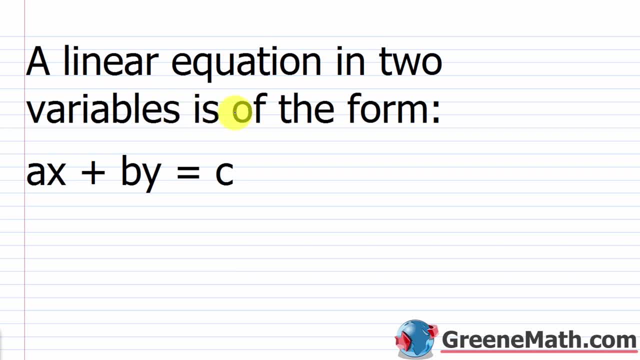 here. so a linear equation in two variables is of the form and we see ax plus by equals c. so the first thing I want to call your attention to is our variable x and our variable y. each is raised to the first power. remember if you have a variable or a number. 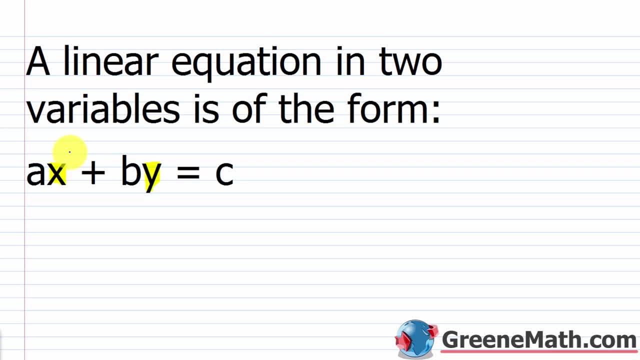 and there's no exponent that's visible, it's understood to have an exponent of one. so I can do this now. if you see, something like ax, squared plus by squared, equals c, that's not a linear equation. okay, so the fact that the exponent is one in each case. 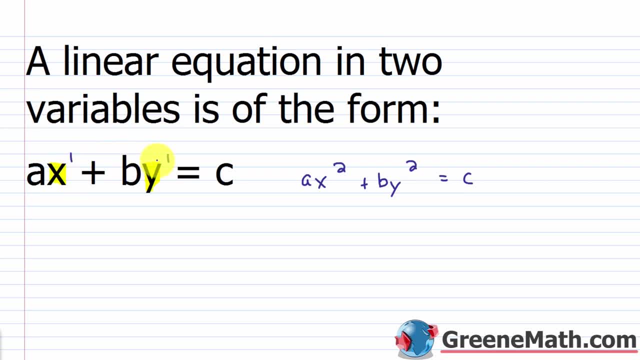 or you don't see an exponent- is what makes it a linear equation. alright, so the next thing that I want to call your attention to, we have this a. let me kind of highlight this in a different color. we have a, we have b and we have c. 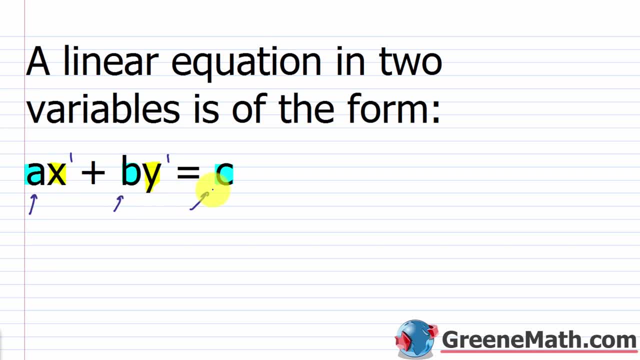 so for each of these we kind of say in our book- and if you're fumbling through a textbook right now, you would see something like a, b and c are real numbers, with one restriction: it's not allowed for a and b to be zero at the same time. so in other words, 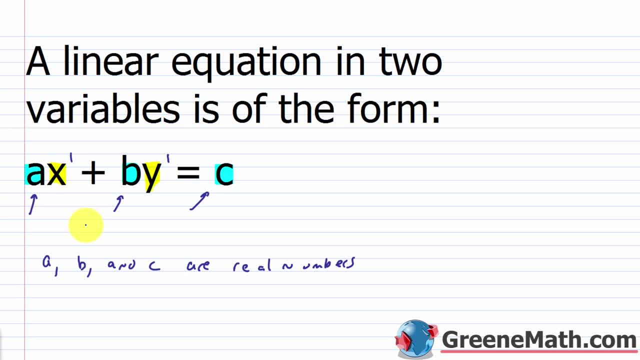 a could be zero if b is not, b could be zero if a is not. but a and b cannot both be zero again at the same time. so I'll just write here that a and b are not both zero. okay, and the reason for that is: if they were both zero. 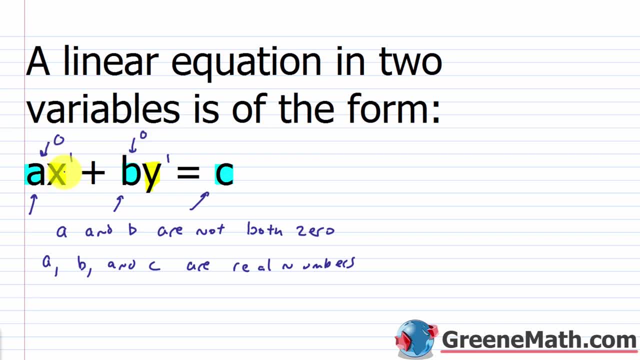 think about if I plugged in a zero here and here. well, zero times x would be zero, zero times y would be zero. you'd have: zero equals c. well, that's only true if c is zero. so your variables would basically drop out right. so what would be the? 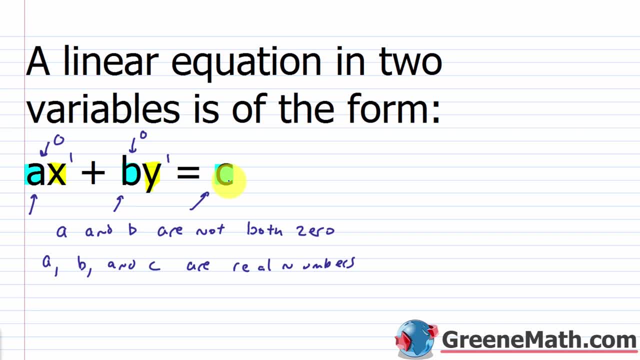 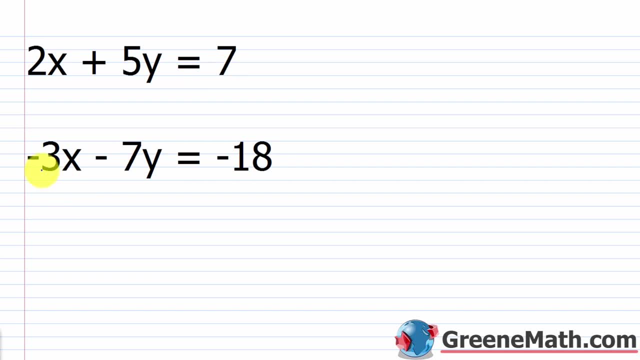 point there. so a and b are not both zero. a, b and c are real numbers. so let's look at two quick examples. so we have two x plus five- y equals seven. we have negative three x minus seven- y equals negative eighteen. so again, in each case you can kind of match. 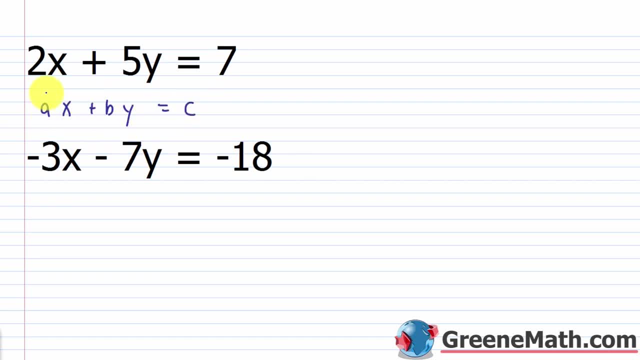 this up with what I showed you as your generic example. so a here is two, b here is five, c here is seven. you have x to the first power. you have y to the first power. if I look at this example below, a is negative three, b is negative seven and c is. 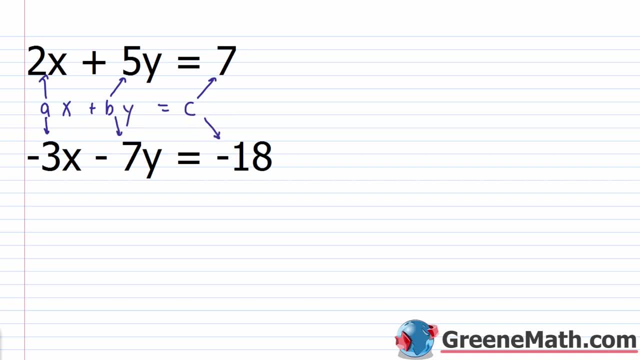 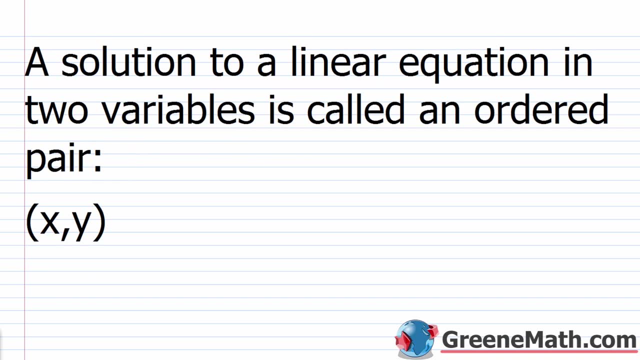 negative eighteen. so very easy to kind of line these up with a generic example and see what we mean when we talk about a linear equation in two variables. alright, so the main thing that's different is that when we work with a linear equation in two variables, it's: 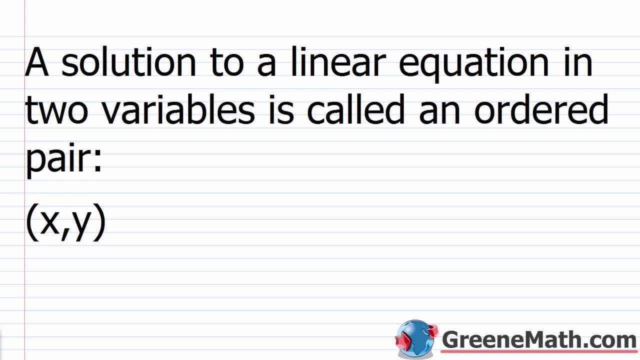 no longer going to be one solution. there's an infinite number of solutions that's going to work. so for this reason, we generally are going to graph our solution set to the equation to give a visual representation of what's going on now. we're not going to graph in this. 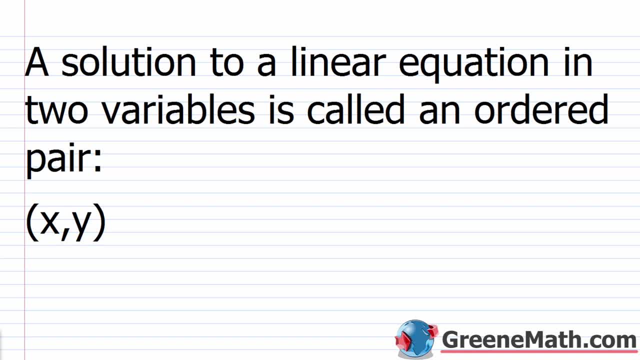 lesson, but we're going to do the things that lead up to us being able to graph, and you know from algebra one- if you took an algebra one course- that graphing is not very difficult. right, it's actually very, very easy. so the first thing we need to understand is something called an. 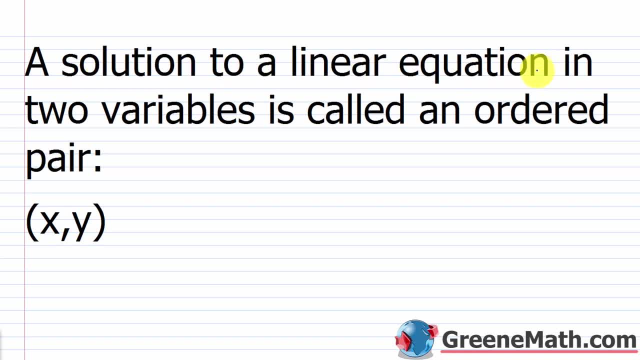 ordered pair. so a solution to a linear equation in two variables is called an ordered pair. so generically we work with x and y. okay, so x is in the first position, so it's always first, and then y is always second. so if i give you an ordered pair like 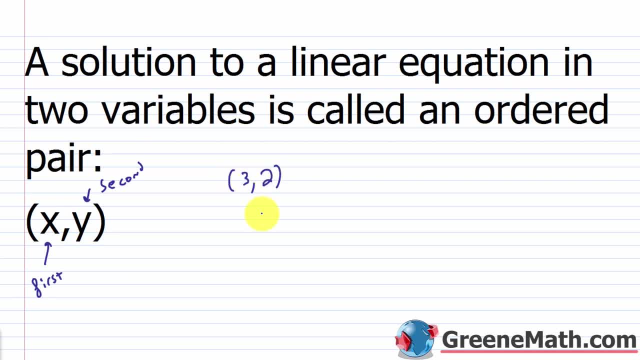 three comma two, and i say it's a solution to a certain linear equation in two variables. that means that i can plug in a three for x and a two for y and i would get a true state: right, the left and the right side would be equal. so the main question: 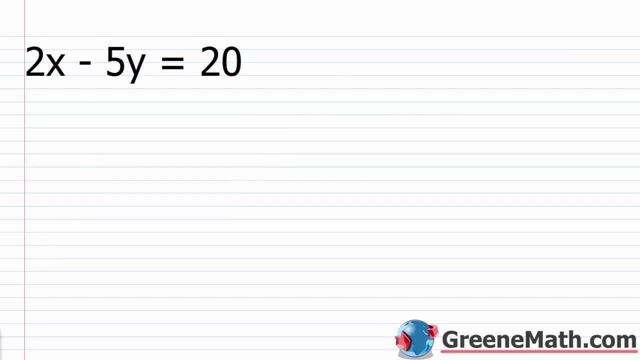 you might be asking right now is how do we get an ordered pair or how do we get such a solution for an equation? well, basically, we pick a number and plug in for one of the variables, and then we solve for the other, so i can pick whatever number i want. 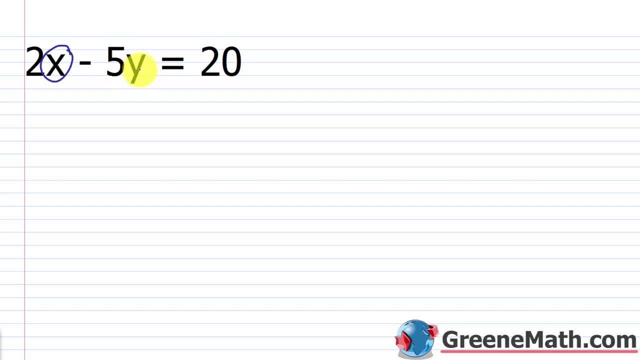 for x and then i can solve for y, or i could pick whatever number i want for y and then solve for x, and there's again an infinite number of solutions. i can choose any number i want and i'll be able to get a solution for the other one. so let's just 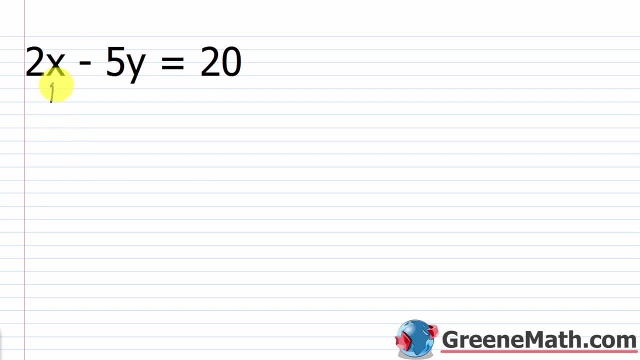 start out with x equals to zero. that's an easy one. so let's say x equals zero. so i would say: two times zero minus five, y equals twenty. and what i'm basically doing is, by plugging something in, i'm creating a linear equation in one variable that 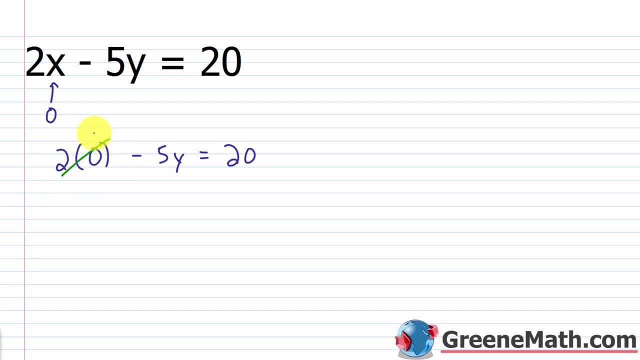 i can solve quite easily. so two times zero is zero, so we'll put zero there. negative five y equals twenty. so we divide both sides by negative five, that will cancel. i'll have y is equal to negative four. so it's important to note what we did here. 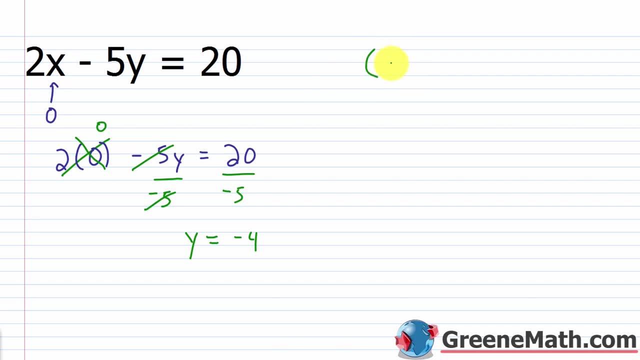 i plugged in a zero for x, so that means this ordered pair here. remember it's x comma y. so it would be a zero for x and it would be a negative four for y and just plug in. let me just erase everything and start from scratch. let's pretend. 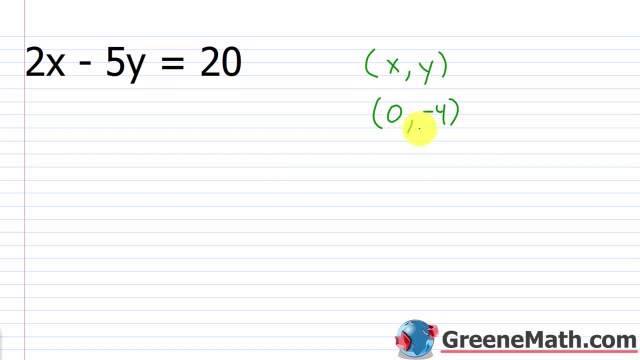 you're given this ordered pair and you say: hey, does this work as a solution? well, i'm plugging in a zero for x- okay, this is my x value- and i'm plugging in a negative four for y. that's all i'm doing. so two times zero. 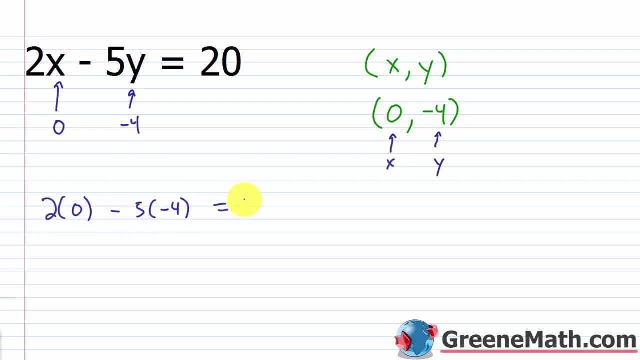 minus five times negative four does that equal twenty. two times zero: again is zero. negative. five times negative four is positive twenty. so yeah, of course this does work. twenty is going to equal twenty. so yeah, that works as a solution. all right, let's just try something else. let's say: i picked some. 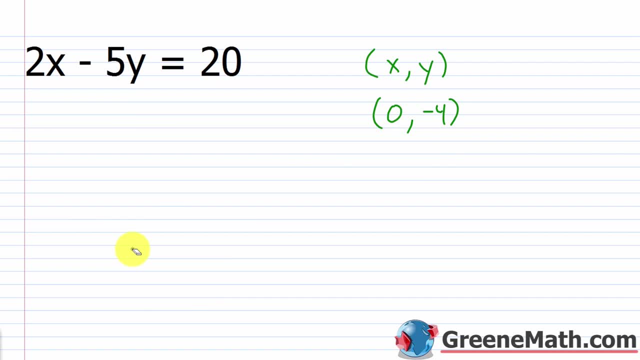 number for y doesn't matter what it is, let's just say six. okay, that's nice and easy, so i plug in a six for y. well, i'll have two x minus five times six equals twenty. so i'm going to evaluate this: negative five times six is negative thirty. 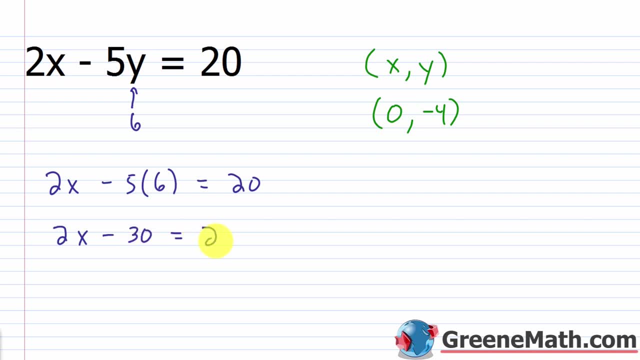 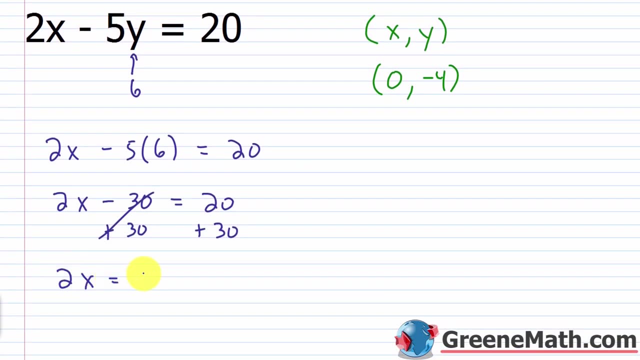 so i'd have: two: x minus thirty is equal to twenty. i would add thirty to both sides of the equation. this would cancel. i'll have two: x is equal to twenty plus thirty is fifty. divide both sides by two and finally i'd find that x is equal to twenty five. 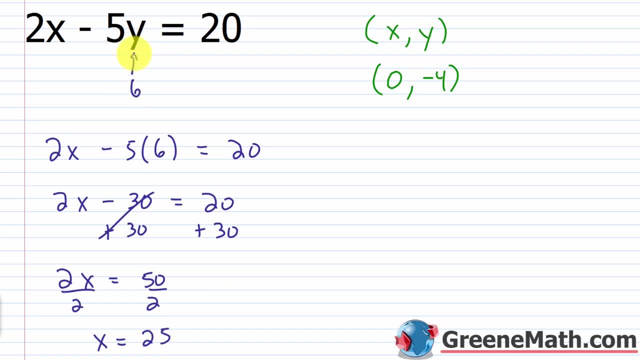 so when y is six, okay, i plugged in a six there to start. x is twenty five. so again, following this format, the x value is first, so that's twenty five, the y value is second, so that's six. and again, i can generate as many of these as i'd like. pick some. 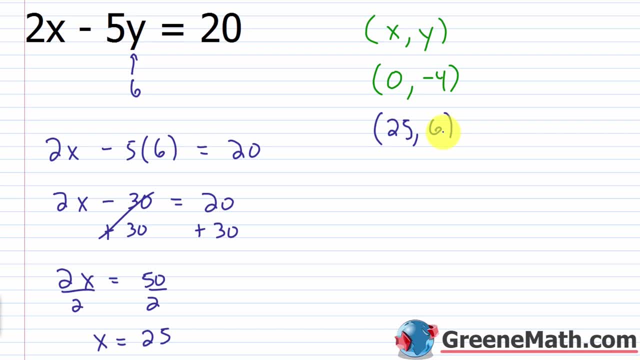 for x, solve for y. pick something for y, solve for x. alright, so let's kind of look at our first kind of sample problem here. this is something you're definitely going to see in your textbook as you get into starting to graph these linear equations in two variables: the 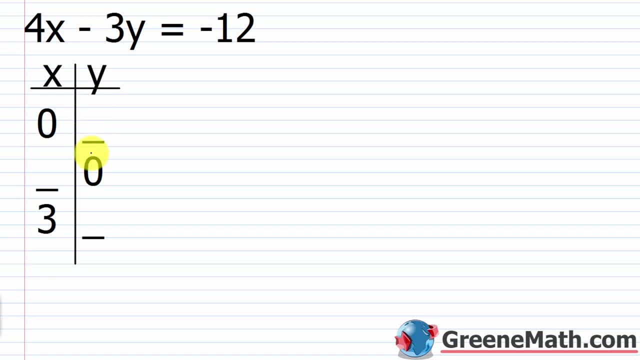 first thing you do, or the first thing you're taught, is how to create a table of values. what this is going to do is it's going to give you some ordered pairs that you're then going to plot on the coordinate plane, and then you'll sketch a line. 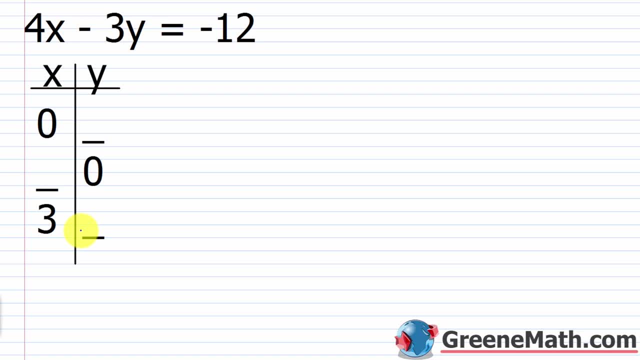 through those ordered pairs to create your graph. well, we're not there yet, we're still working on this, but i just want you to know where we're going. so we have four x minus three y equals negative twelve. now i'm given a table with some values filled in for me. 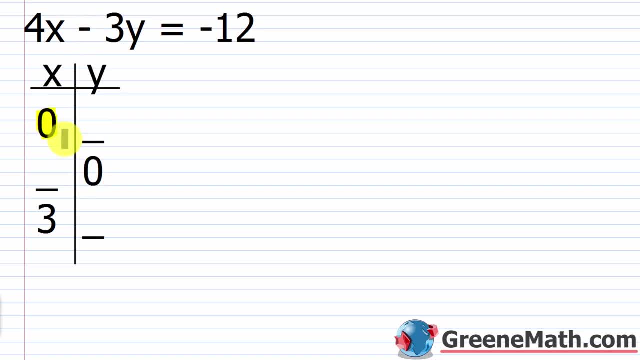 so, for example, i'm given an x value of zero here. so what they're saying for me to do here is to take this equation. so four x minus three y equals negative twelve. plug in a zero for x and see what i get for y, so four times zero. 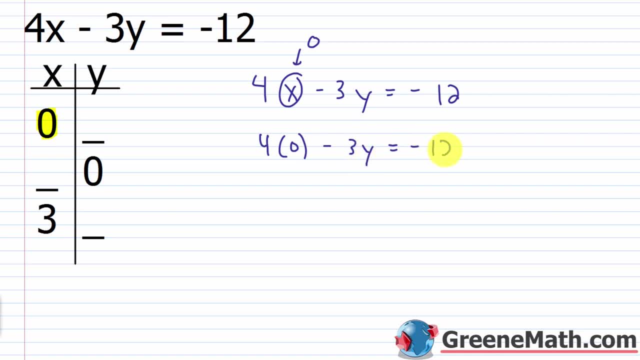 would obviously be zero minus three. y equals negative twelve. so this is gone. basically, all i need to do to solve this is divide both sides by negative three. that would cancel and i'd have y is equal to four. so i can fill in my missing part here and put a four there. 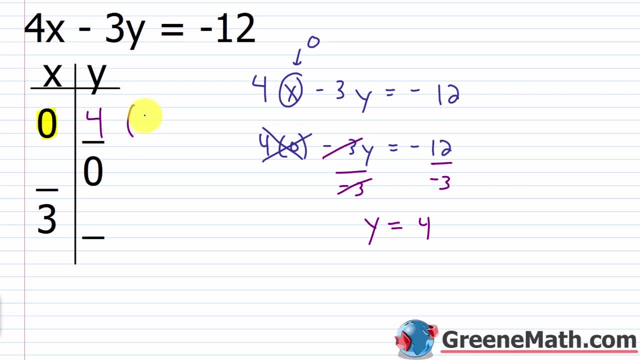 so the ordered pair: there would be zero comma four. again it's the x value first, followed by the y value second, and just write that down in your notes. just put x comma y so you can refer to it as we're doing this and this is something you're going to remember. 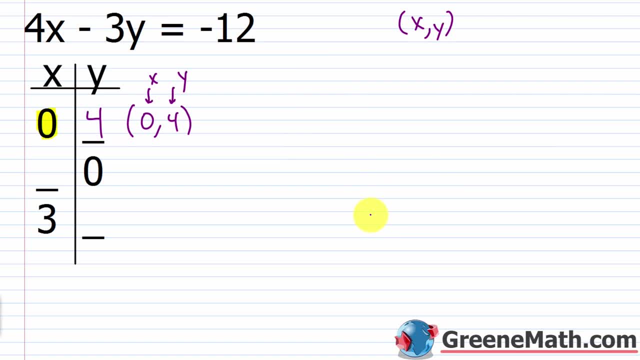 for the rest of your life. x comma y is the ordered pair. alright, for the next one we're given a y value of zero. so for the y value of zero i go four x minus three times zero. just plug in a zero there, which corresponds to right here. 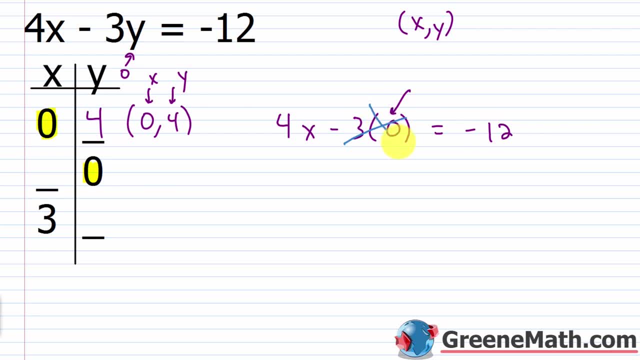 equals negative twelve. three times zero is obviously zero, so that's gone. so we'll have four. x is equal to negative twelve. let's divide both sides by four, that'll cancel, and we'll have: x is equal to negative three. so when y is zero, x equals negative three. 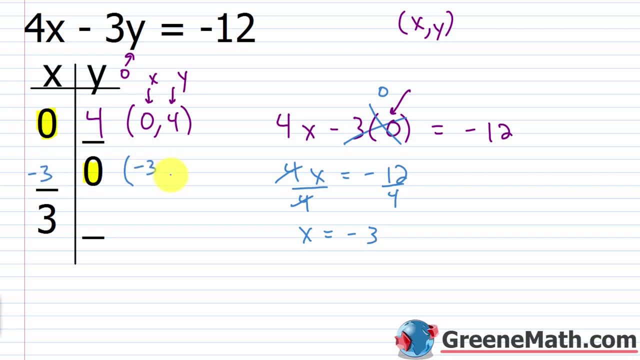 again as an ordered pair. x comes first, so that's negative three comma. y goes second, so that's zero. so this is your x, this is your y. alright, let's take a look at one more. so now we're given an x value of three, so let's plug that in. 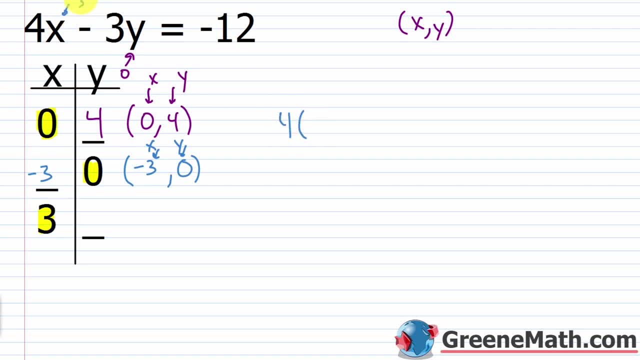 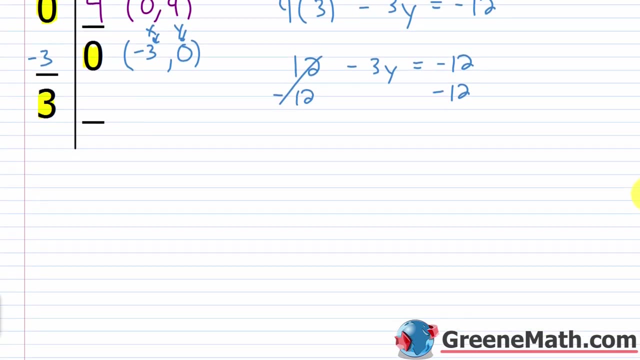 so we have four times x. again, i'm plugging in a three. that's all i'm doing. then minus three, y equals negative twelve. four times three is twelve. minus three y equals negative twelve. let me subtract twelve away from each side, so that cancels. scroll down to get a little room. 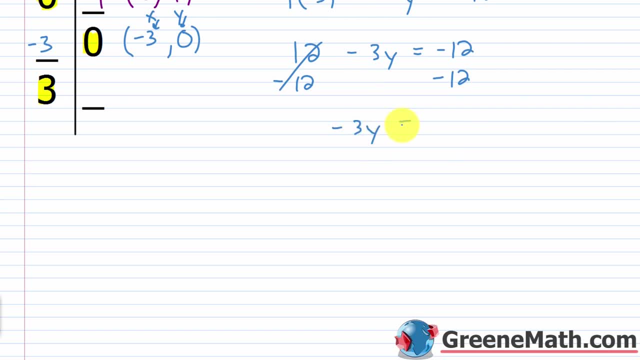 so then i'd have negative three. y on the left is equal to negative. twelve minus twelve is negative twenty four. divide both sides by negative three, so this would cancel and i'll have y is equal to eight. so when x equals three, x is three, y is eight. 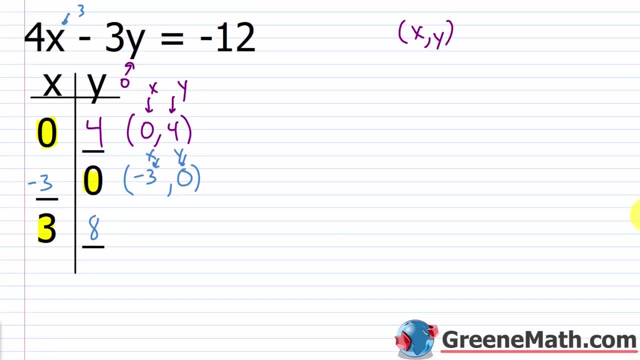 let me erase this so we can get everything back on the screen. let me scroll up here. so, as an ordered pair, this would be three for x, comma eight for y. so this is x and this is y. so pretty simple exercise overall. for sure you'll probably get this on your. 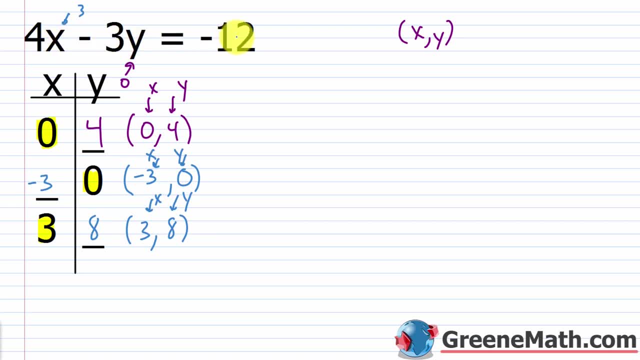 homework or on a test, where they give you a linear equation of two variables and they'll either tell you to make a table with a certain number of ordered pairs or they'll give you an ordered pair where the x value or the y value is missing, like we did here. 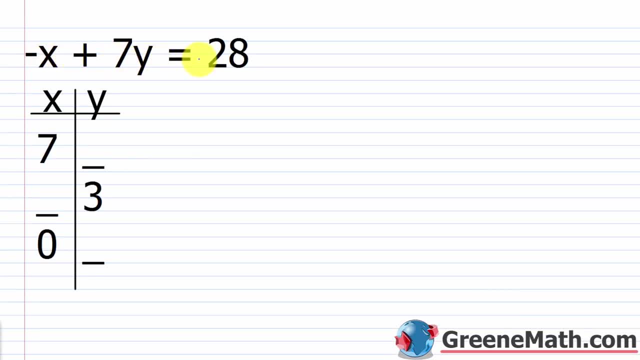 alright, let's take a look at one more of these. so we have negative x plus seven y equals twenty eight. so i'm given my table of values. i have x values and i have y values. so the first one gives me an x value of seven. so i'm going to plug that in there. 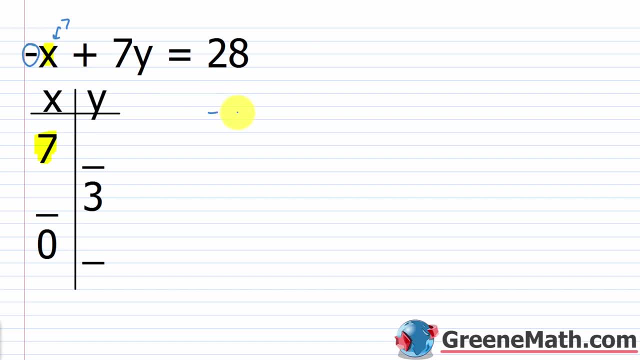 plug in a seven there, don't forget that negative. so put the negative and then plug in a seven plus seven y equals twenty eight. let's add seven to each side, so that cancels. we'll have seven. y is equal to thirty five. we'll divide both sides by seven. 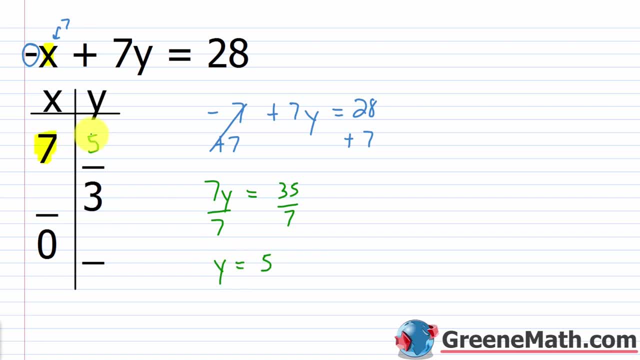 we get: y is equal to five. so when x is seven, y is five. okay, so let me erase this. and that's the ordered pair. remember: the x value is first, so that's seven comma. the y value is second, so that's five, so this is x. 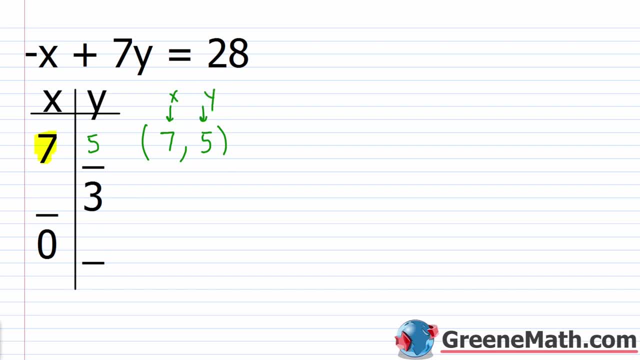 and this is y. alright, for the next one, we are given a y value of three. so we're going to plug in a three here and we're going to solve for x. so we have negative. x plus seven times three is equal to twenty eight. let me. 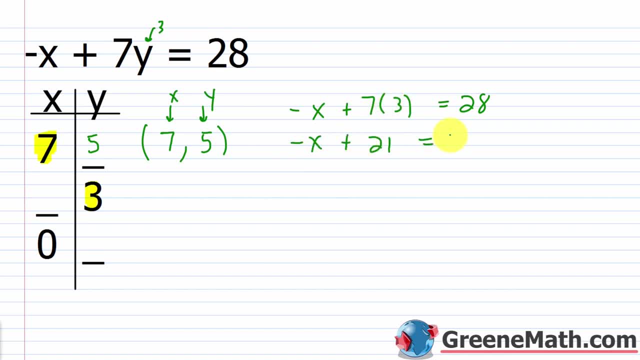 say that seven times three is twenty one. so negative x plus twenty one equals twenty eight. let me subtract twenty one away from each side of the equation, so this is going to cancel. we'll have: negative x is equal to twenty eight minus twenty one is seven. we'll divide both sides by 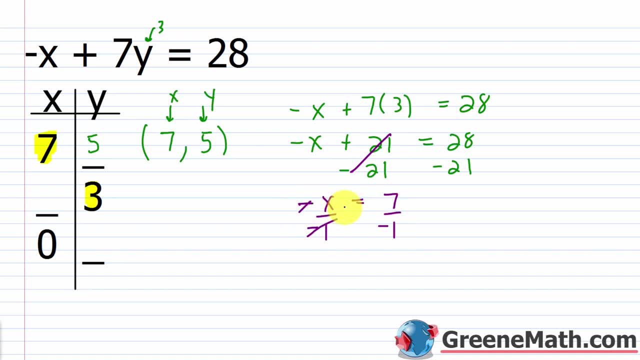 negative one or multiply by negative one, whatever you want to do, so that will cancel itself out and i'll have: x is equal to negative seven. so when y is positive three, x is negative seven. so as an ordered pair, you can write this as negative seven for the x value. 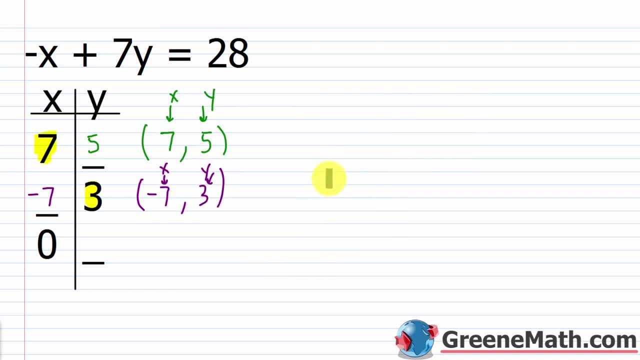 comma three. for the y value, alright. for the next one, we're given an x value of zero. so i'm going to plug that in right there. okay, i want a zero there, so negative. and then you have zero plus seven. y equals twenty eight. the opposite of zero is just zero. 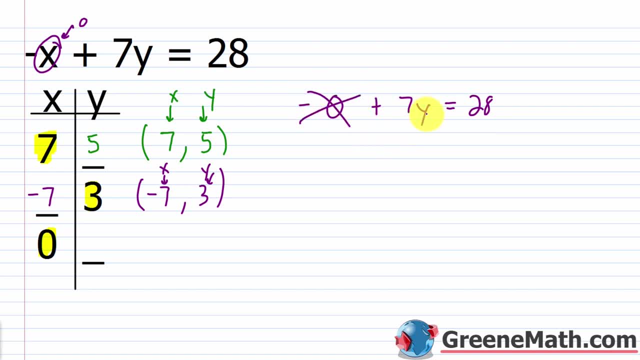 so this? you just cancel that out and say: i'm just dealing with seven. y equals twenty eight. we would divide by both sides by seven and we would find that y is equal to four. so when x is zero, y is four. so we have zero comma four. 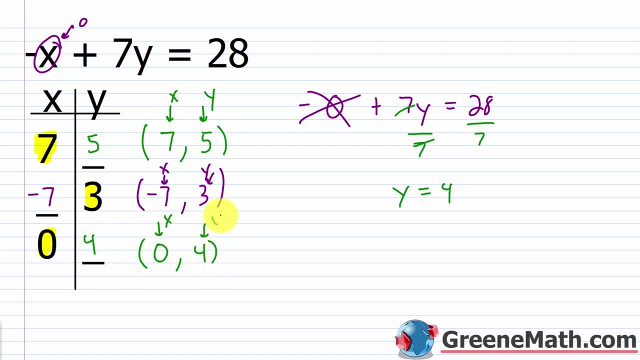 again, zero is the x value, four is the y value. so pretty simple exercise overall. not going to do any more of these for now, but you can pretty much tell what you need to do. if you're given an x, you plug in for x in that equation. 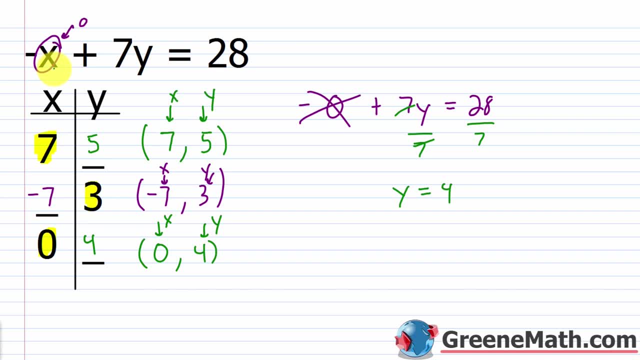 and you solve for y. if you're given a y, you plug in for y in that equation and you solve for x and then just report your answer as an ordered pair. remember the x value goes first comma, your y value. so kind of the next thing we need to learn. 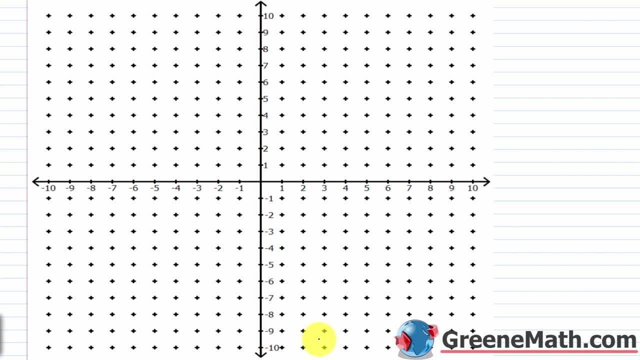 before we start graphing these linear equations in two variables is what to actually do with the ordered pairs. what's going to happen is we're going to end up plotting them on something known as the coordinate plane. so this is the coordinate plane, and for those of you again, that took 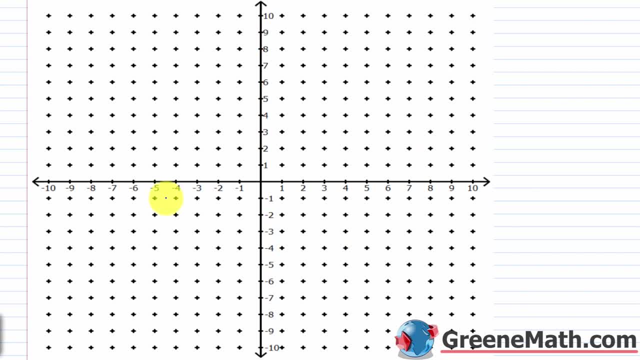 algebra one. you're very familiar with this. we did a lot of work with this in algebra one, but if you've never taken that course, this is new to you, so let me give you a couple of tidbits of information here. the first thing is that this thing has many names. 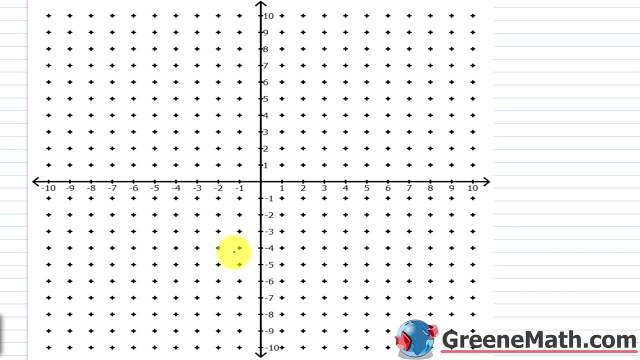 the official name for it is the cartesian coordinate system and it's named after a guy that was sick in his bed and he watched a fly kind of go back and forth. so he came up with the idea for this. the other name you might hear is the rectangular coordinate. 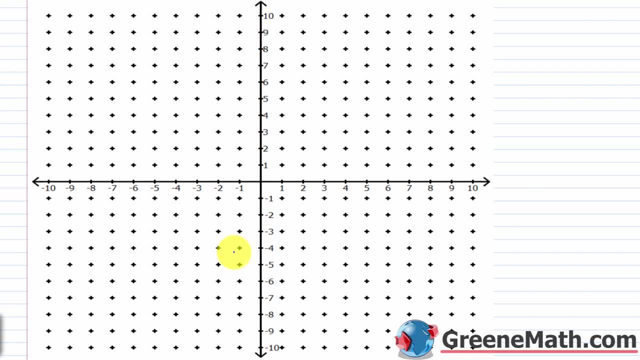 system, but most often I think that you'll hear it called the coordinate plane. but it's interesting to know those three names because those are used most often and if your book uses something different, I don't want you to be confused. what was he talking about? he said coordinate plane. 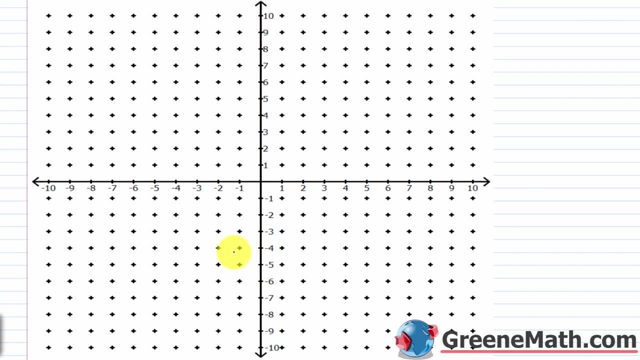 they're calling it this cartesian thing, so it's important to kind of know other names for it so you don't get confused. the other thing would be: how does it work? well, it's two number lines basically that intersect where they're each at zero. so this is the intersection. 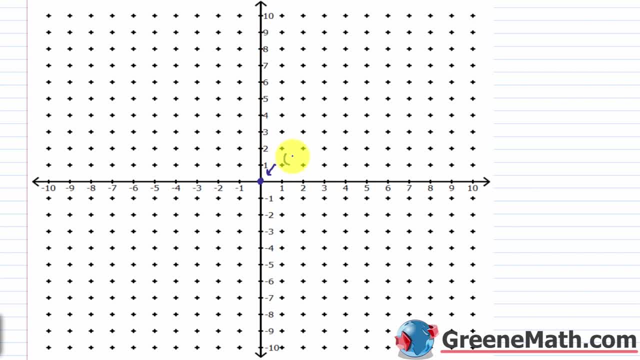 of the two. it's the point zero, comma zero, so the x value is zero, the y value is zero and it's again the intersection of the two. this is referred to as the origin, and you're going to hear that a lot throughout your study of mathematics. 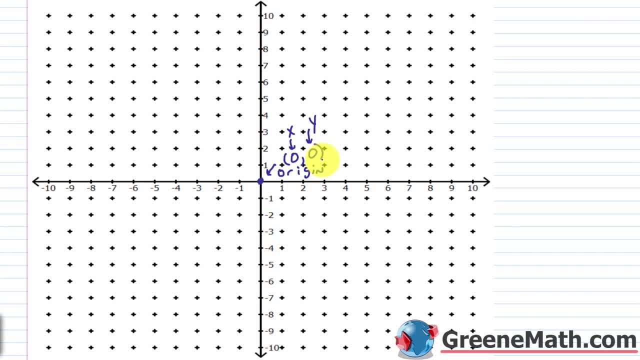 whenever you talk about the coordinate plane, somebody refers to the origin. they're talking about this point right here: zero comma zero. now, another thing that's important is the horizontal number line is referring to x locations, so we refer to this as the x axis now. similarly, the vertical axis refers 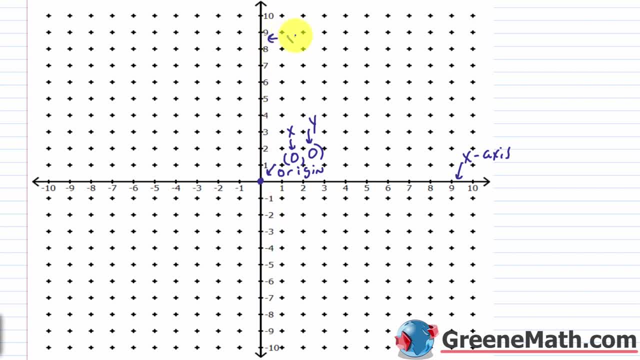 to y locations. so this is referred to as the y axis. and to plot an ordered pair is very, very simple. if I give you something like four comma three as an example. this is your x value, this is your y value. so that just translates to finding the x location of. 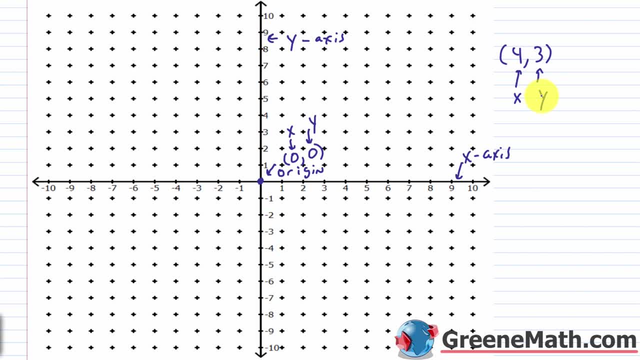 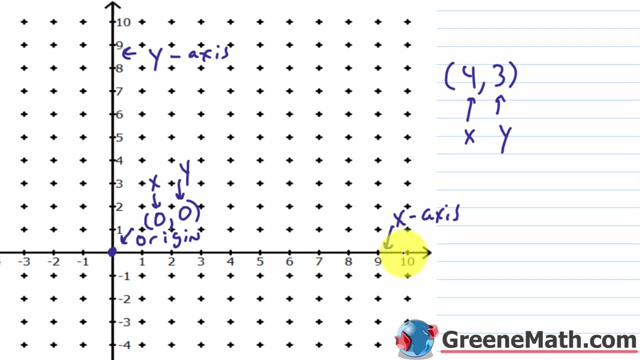 four, finding the y location of three and just getting the meeting point. so an x location of four. I look at the x axis again, the horizontal axis, so I go from the origin one, two, three, four units to the right, or I could just start at four either way. so 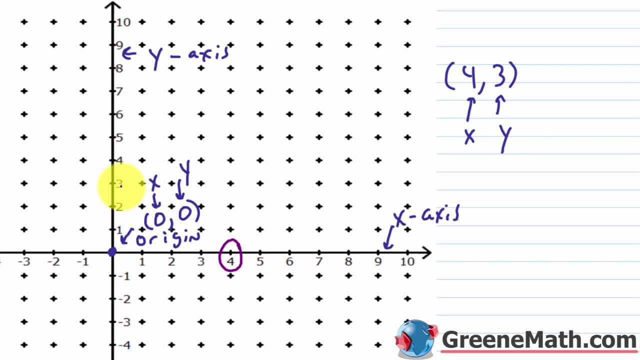 that's an x location of four, a y location of three. I just go up three units to right here and where's the meeting point? well, I would go one, two, three, four units to the right and I would travel one, two, three units up. it's right there and it works. 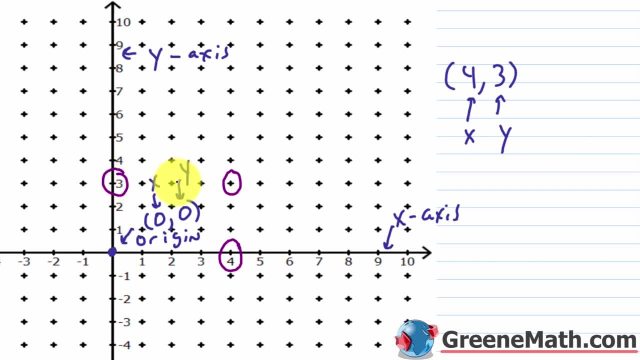 either way, if I want to go one, two, three units up and then one, two, three, four units to the right, I get to the same location. so this is the point, which I'll label four comma three, and four comma three is known as the coordinates of the point. it tells us: 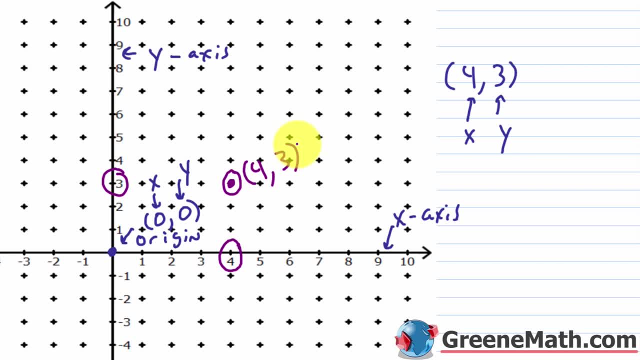 where to go right. we go four units to the right and three units up to get to this point. now just one more piece of information before we look at some examples of plotting ordered pairs. you're probably taught in your textbook- and this is very brief- about the quadrants. 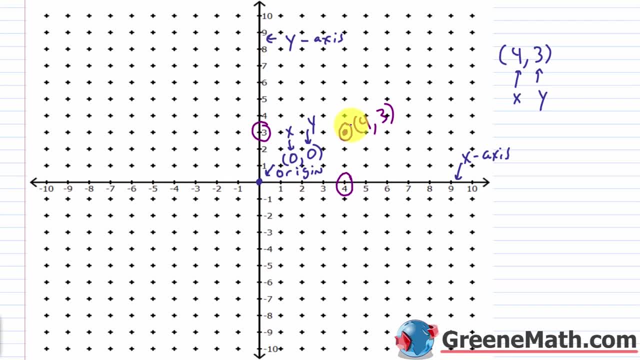 so the quadrants go counterclockwise. so you kind of think about each section here. this is section one or quadrant one, so that encompasses this. this is quadrant one, and then you'd have quadrant two. let me do that in a different color. so this is: 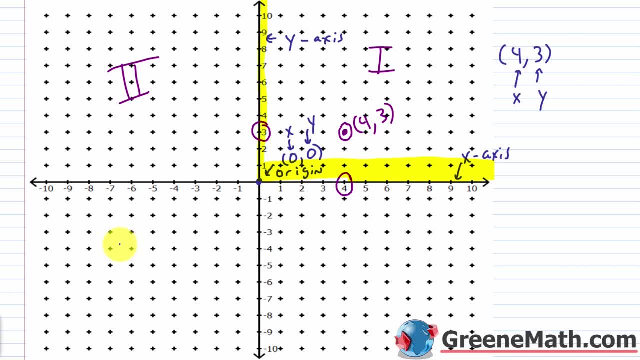 two and this is three and this is four, so again counterclockwise, so you can highlight this in a different color. this is two. I'm trying not to go over the line. I know I'm terrible at drawing, but I'm trying. and then let's. 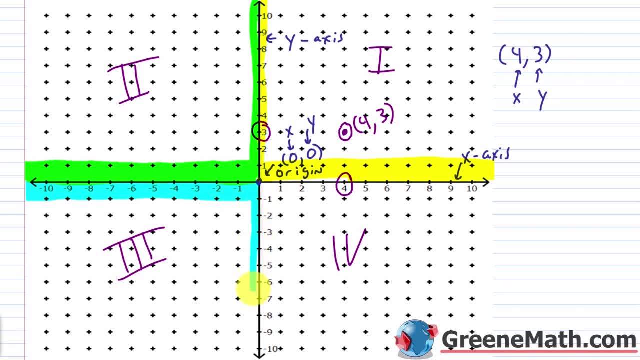 do this one in a different color. this is three, and then one last color. let's do orange for four, and I know again I went over the line in a couple places, but you should get the idea. so quadrant one just in here encompasses all of this right and it extends forever and ever. 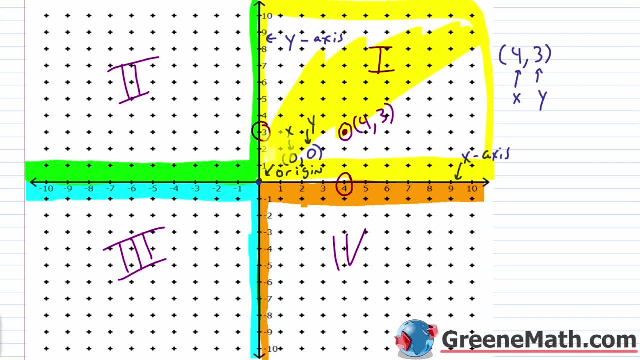 and ever in this direction. right, it goes forever, but it's all the values that would be in here. and one of the things we can say about quadrant one is what? well, we know that the x location and the y location are each going to be positive, because anything in this quadrant here 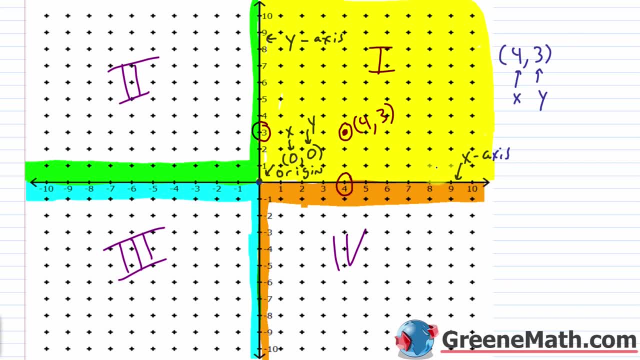 you can see highlighted in yellow, is going to be to the right of zero and it's going to be on top of zero, moving up from zero. so the direction going to the right is positive, the direction going up is positive. so anything in quadrant one is positive, positive. 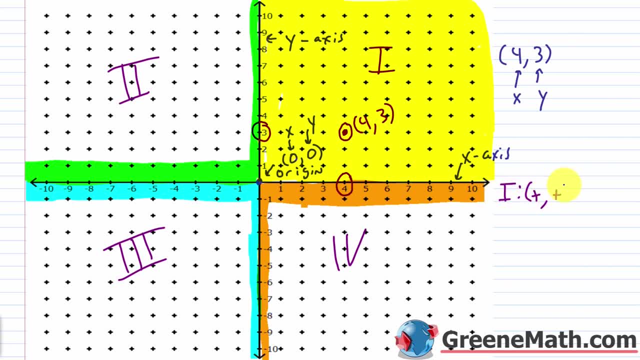 so quadrant one is positive. positive, so this is your x and this is your y. for quadrant two, what can you say? well, the x locations are going to be negative. the y locations are positive, because we go to the left of zero and we go north of zero. 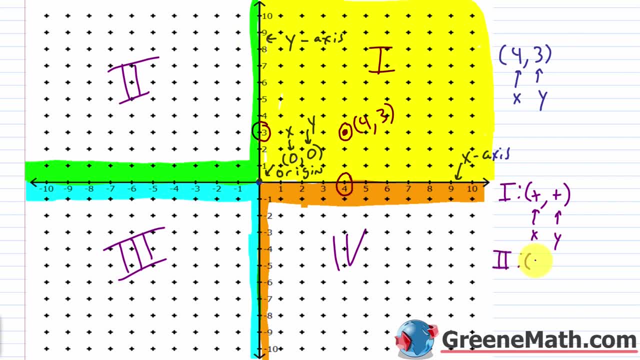 so that's going to tell me that in quadrant two, again, my x location is negative, my y location is positive. in quadrant three, I am negative and negative because my x location is to the left of zero, my y location is south of zero. so for quadrant three, 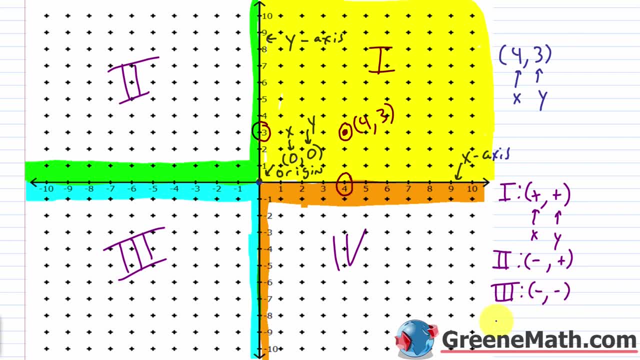 I am negative, negative. and then, finally, for quadrant four, I am positive in the x values because I'm right of zero, and then I'm negative in y values because I'm south of zero. so this is positive, negative, and you might be tested on something like this: 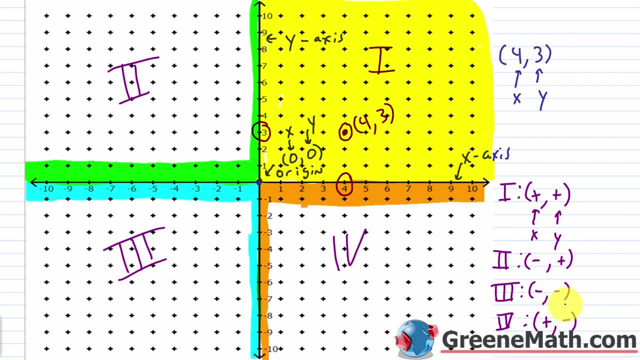 it might say, for example, what are the values in quadrant two? and you might get flustered and say, well, I didn't memorize that, you don't need to just draw yourself a sample coordinate plane. they're very easy to draw and once you do that you can just eyeball it. 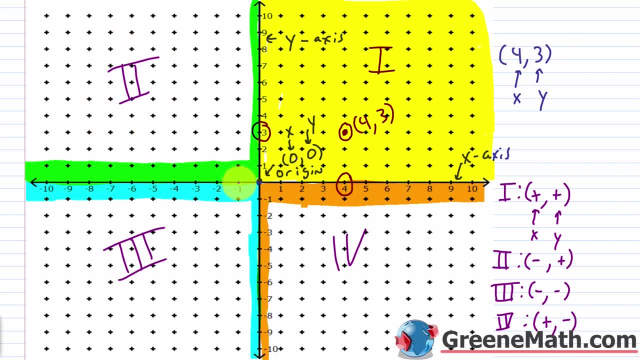 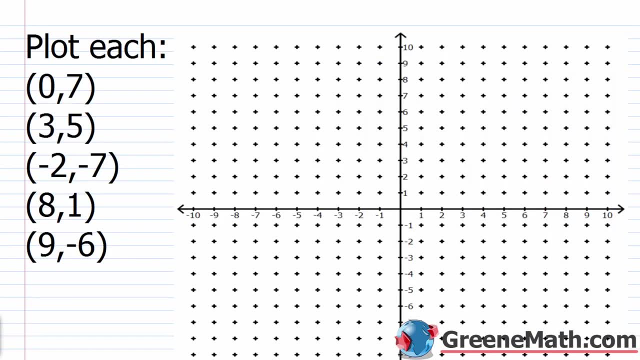 and say: well, I know that anything in quadrant two would be to the left of zero and north of zero, so my x values would be negative, my y values would be positive. alright, so let's wrap up this lesson and we're just going to plot some ordered pairs. 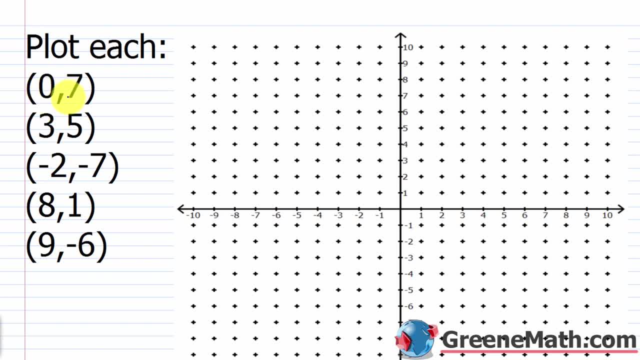 so we're going to start out with zero comma seven. so again, it's x location, followed by y location. so let me just write this real quick: it's x comma y, and let me just label this too, so that we don't get confused. this is the y axis. 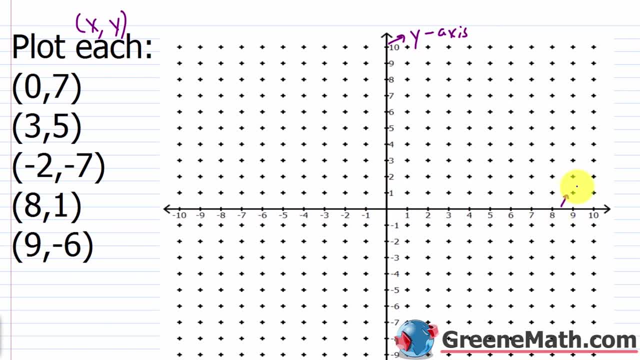 and this let me kind of scroll over: this is your x axis. now an x location of zero is not confusing. a lot of you get confused with this. if I look at the x axis, just kind of block out the y axis for a second, just pretend this isn't here. 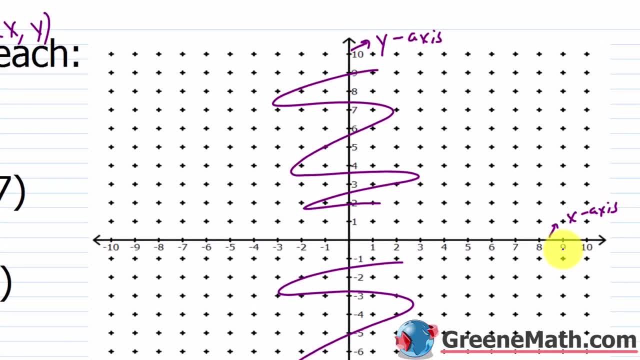 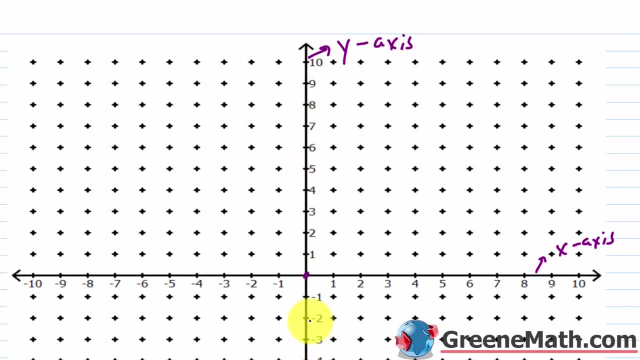 if I have a regular number line we've been working with forever and ever and ever. where is zero? it's right here. so where is seven as far as a y location? now we can erase this and think about seven. it's right here. so if I go, zero units on the x axis. 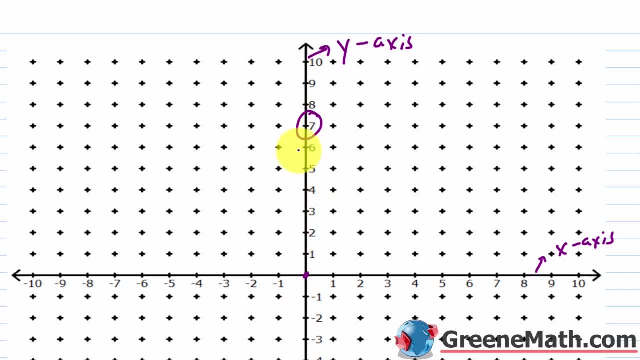 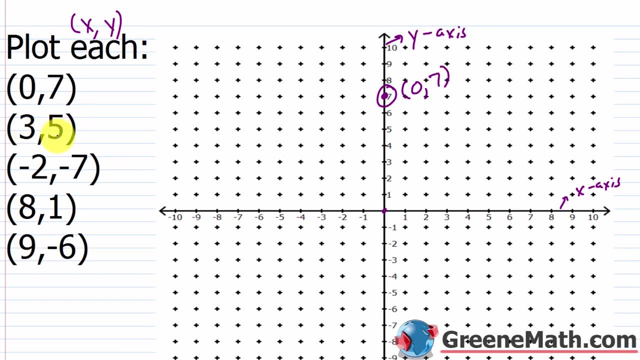 I just don't move. so if I go seven units up on the y axis, I'm right here. so this is going to be zero comma seven. now for the next one. I have the ordered pair three comma five. so I would go three units to the right. 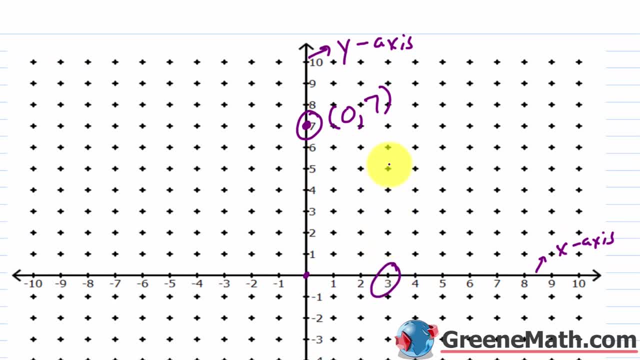 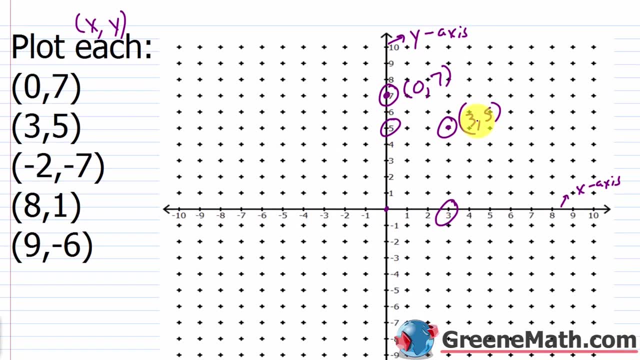 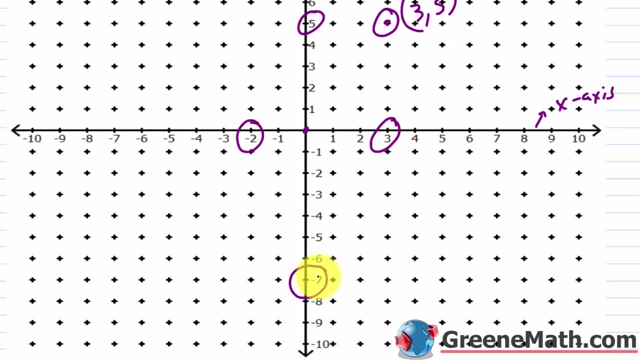 or an x location of three and five units up. one, two, three, four, five. so that's a y location of five. so this is three comma five. what about negative two comma negative seven. so I go two units to the left. here's negative two. I go seven units down. 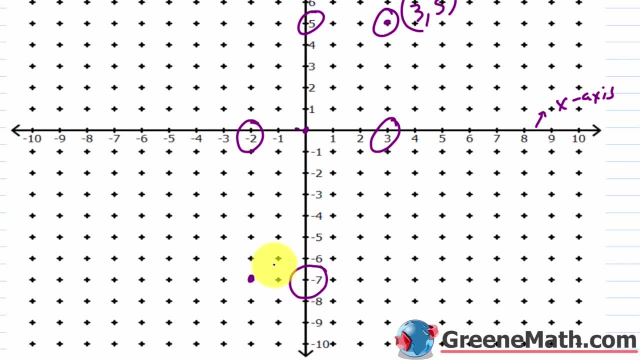 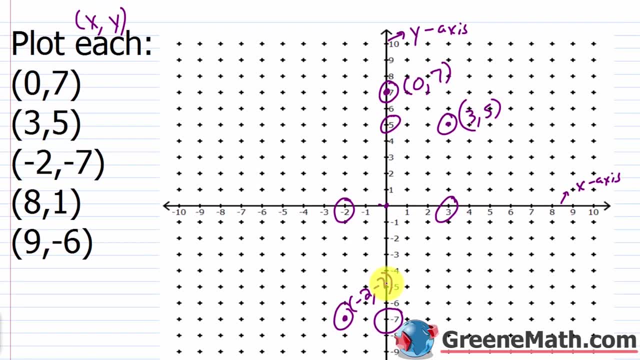 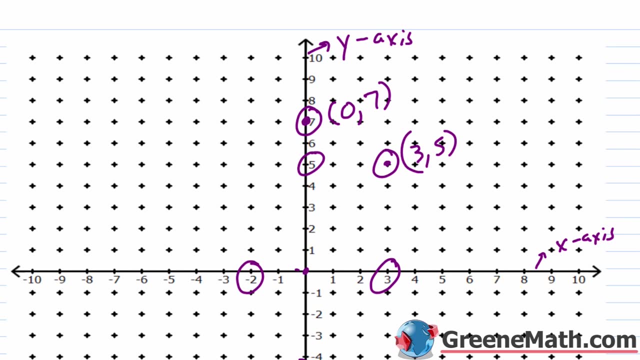 so two units to the left, seven units down is right here. so this is negative two comma, negative seven. next we have eight comma one. so I would find eight on the x axis. let's do this one backwards again. you can do the y location first if you want. 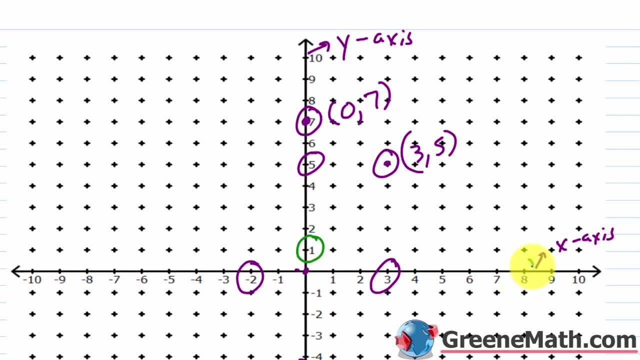 so let's find one on the y axis. that's here. now let's find eight on the x axis. that's here. so let me go up one, and to the right eight. so this is eight comma one, alright. lastly, we have nine comma negative six, so I'm going to find nine on the x axis. 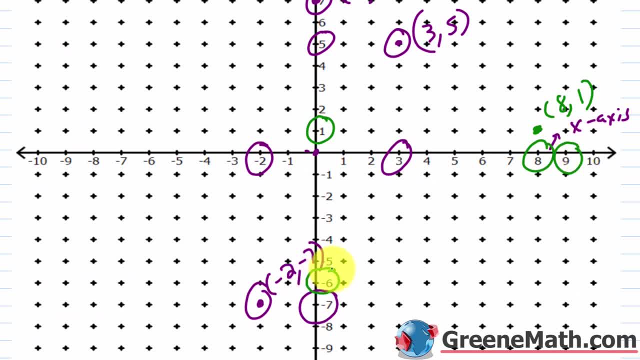 that's here, negative six on the y axis. that's here. so I'm going nine units to the right and six units down. so that's going to be right here. so this is nine comma negative six. so very, very easy in terms of things that you will. 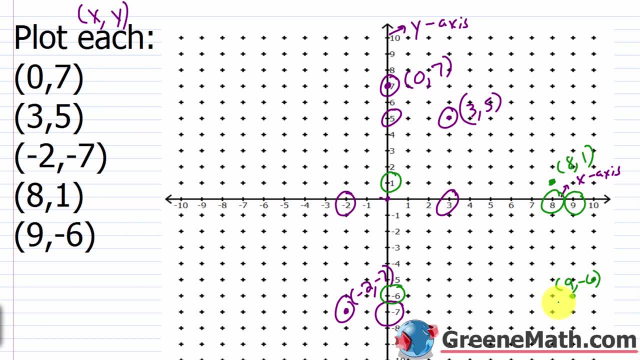 come across in algebra. this is probably one of the easiest things to do to plot an ordered pair. you literally just go to the coordinate plane and have to memorize two things: the x axis and the y axis. the x axis is horizontal, the y axis is vertical. 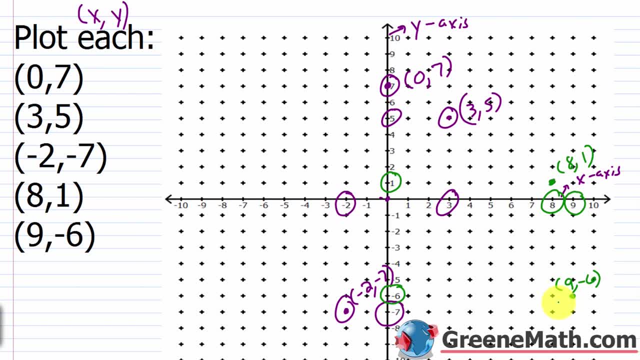 you do that just a few times and you've got that down. so basically, it's just a matter of finding the meeting point of the x location and the y location, putting a little dot there and in most cases, when you're plotting ordered pairs, you just ask you to label it like we did here. 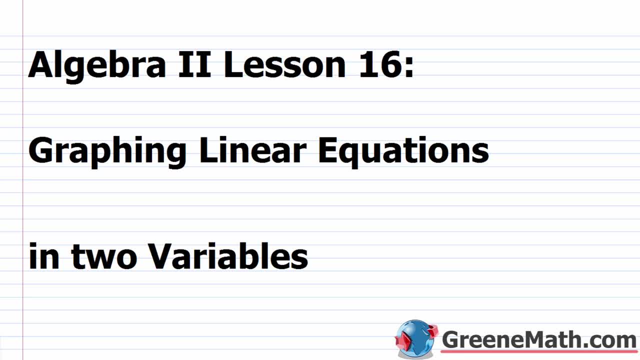 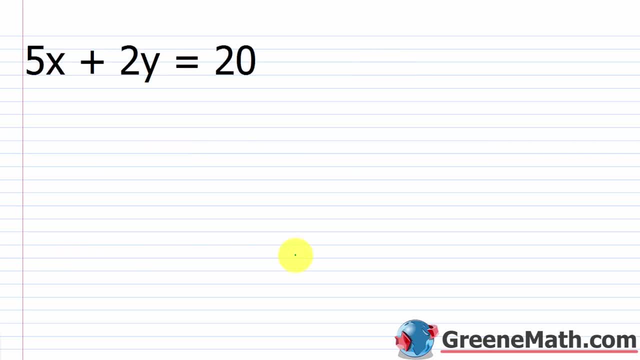 hello and welcome to algebra 2, lesson 16. in this video we're going to learn about graphing linear equations in two variables. so in our last lesson we covered the basics of a linear equation in two variables and if you took an algebra 1 course, 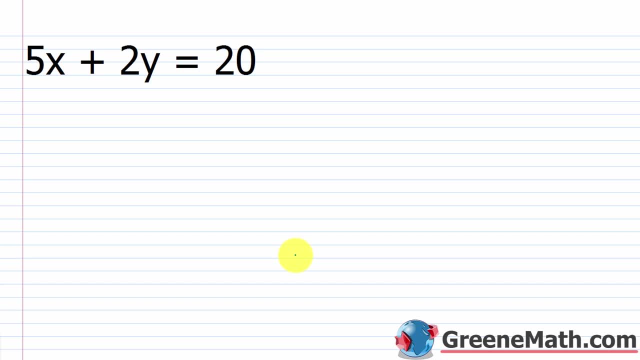 not only was that a review, but this will be a review as well. learning how to graph a linear equation in two variables is very, very simple, particularly if you've done it before. so I want to kind of just start out by covering some of the things we talked about. 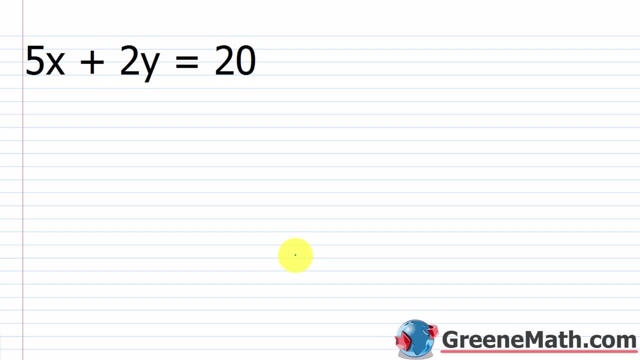 in the last lesson. we're going to go through them very quickly and then we're going to ramp up and start doing some graphing. so a linear equation in two variables looks like this: ax plus by equals c, where a, b and c represent real numbers and a and b are not both 0. 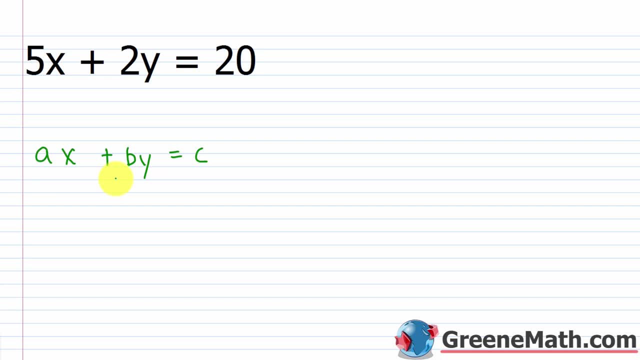 so a can be 0, b can be 0, but they're not both 0. so in this example, 5x plus 2y equals 20. you can see a represents 5, b represents 2 and c represents 20. now another key point here: 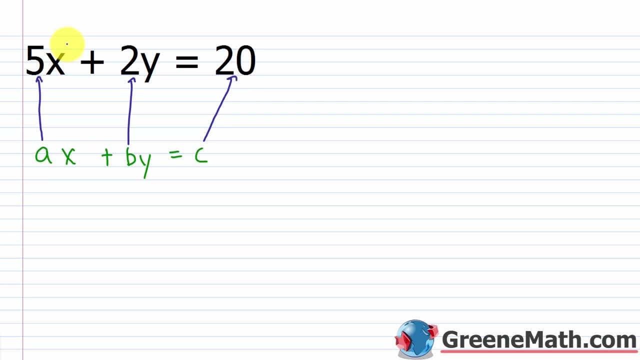 is that the exponent, when each variable is a 1 plus 2y to the first power, equals 20. I would not have a linear equation if the exponents here were something like 2 or 3, for example. so with that behind us, now let's talk about. 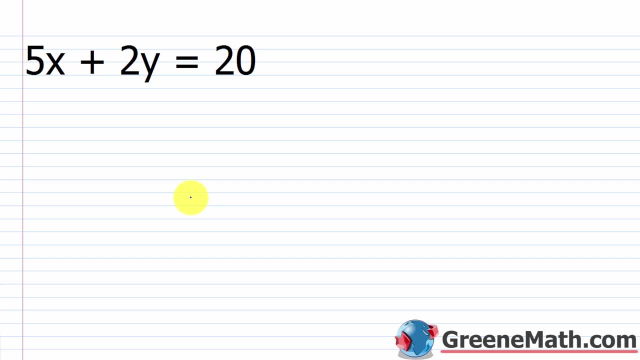 a couple of things with a linear equation in two variables. the first thing is that there's an infinite number of solutions. I can choose a value for x. let's just say 0, for example. I plug it in, I'd have x times 0 plus 2y equals 20. 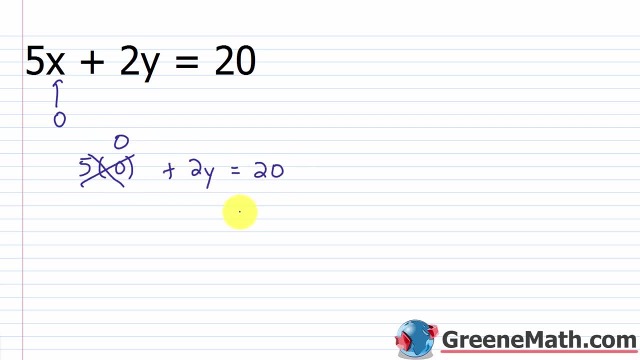 well, this is 0. now I have a linear equation in one variable. I have 2y equals 20. I know that x is 0 because I plugged a 0 in to start. I just need to find out what is y when x equals 0. 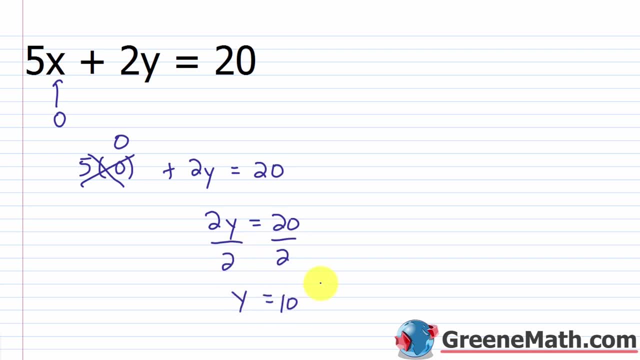 so I divide both sides by 2 and I get y equals 10. so one solution of the infinite number would be that x is equal to 0 and y is equal to 10, and if you want to, you can plug in a 0 for x. 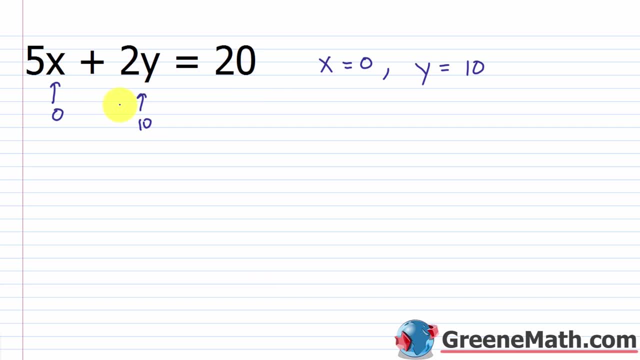 and a 10 for y, you'll see you get the same value on the left as the right. let's do that real quick: 5 times 0 plus 2 times 10 equals 20. this is 0 plus 2 times 10 is 20, equals 20. 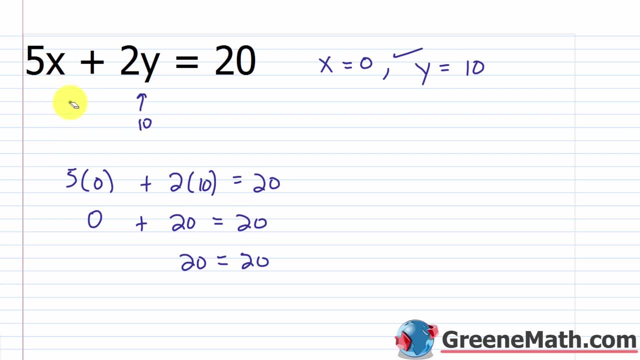 you get 20 equals 20. so this checks out. but the main thing here is to realize that I could choose a different value for x and I would get a different value for y. so let's say, for example, I chose the value of 2 for x. 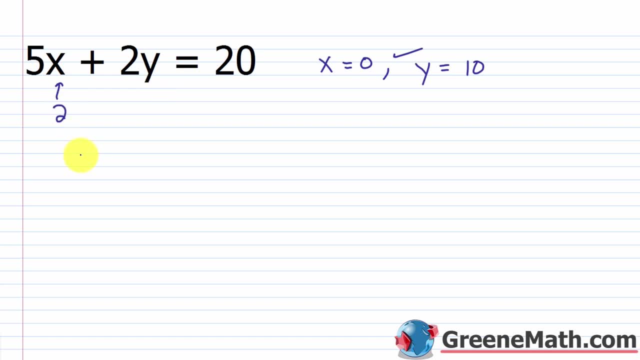 so I plug that in now. so 5 times 2 plus 2y equals 20. 5 times 2 is 10. so this is: 10 plus 2y equals 20. subtract 10: away from each side of the equation, this cancels. 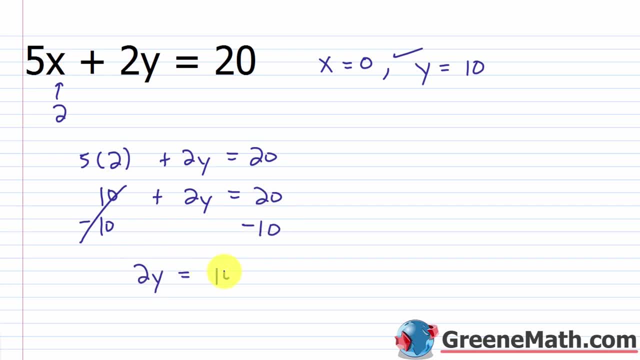 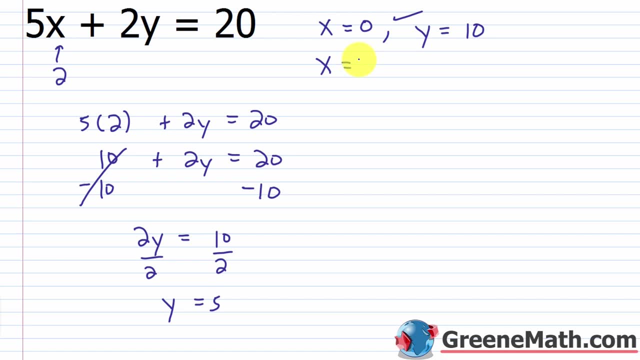 I'll have. 2y is equal to 20 minus 10 is 10. divide both sides by 2, y equals 5. so here x equals 2 when y is equal to 5. so this is a big change for us, because we're used to solving. 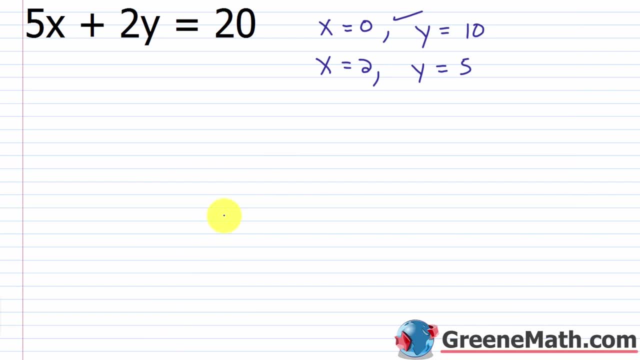 linear equations in one variable, and with those type of equations we generally just have one number that works as a solution. we don't have an infinite number of solutions that we can just generate. but it's good to see this because it leads me to my next point. 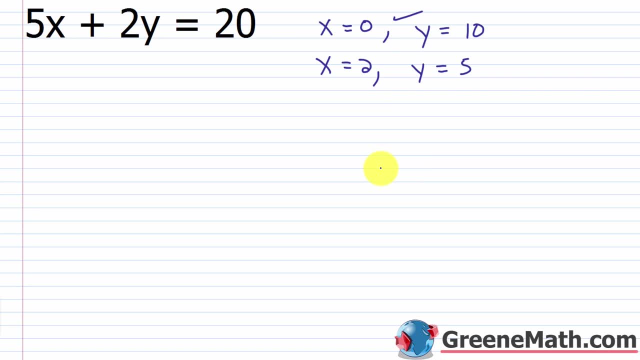 if you have an infinite number of solutions. this is a way to kind of visualize the solution set. and what we do with this is we graph. we graph a line on a coordinate plane to kind of say: hey, here's a visual representation of the solutions for this linear equation in two variables. 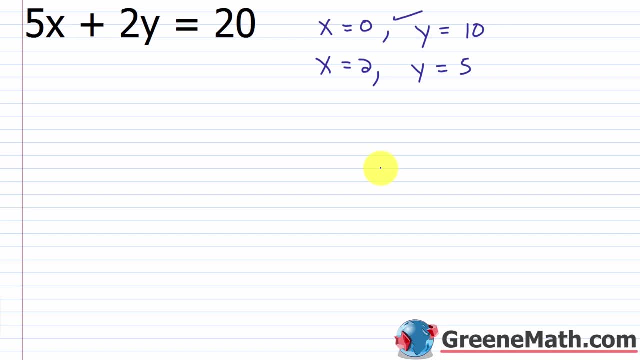 now let's talk about how we would go about graphing something. the first thing is that each solution can be written as something known as an ordered pair, so we talked about that in the last lesson. ordered pair is x, comma, y, so the order is important. I put my x value first, followed by y. 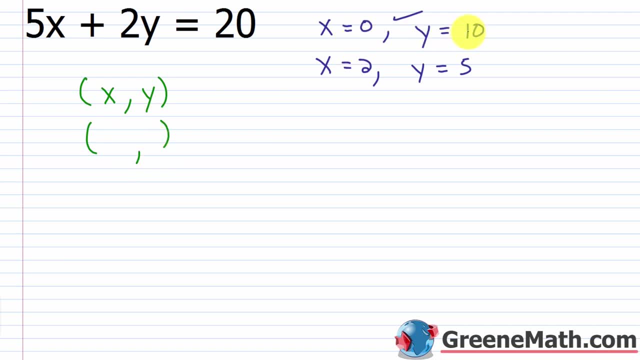 so with x equals 0, y equals 10, the ordered pair would be 0, that's my x value comma, and then 10, because that's my y value for this one. it would be 2 comma 5, and I could generate more if I wanted to. 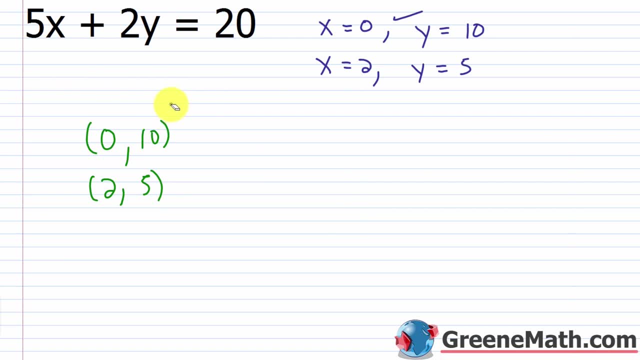 and let's generate one more. actually, let's see what happens when x equals 4. so x equals 4, what is y? so plug in a 4 there we'd have 5 times 4 plus 2y equals 20. we know that 5 times 4 is 20. 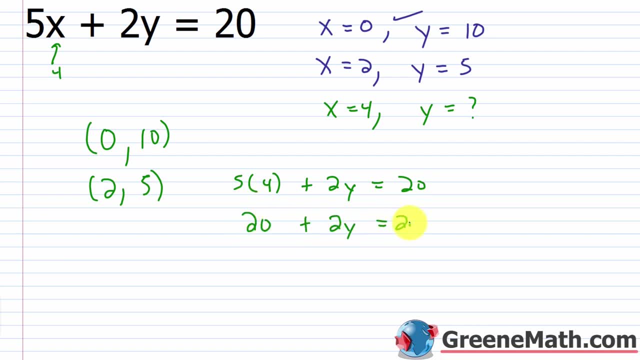 so you'd have 20 plus 2y equals 20. let's subtract 20 away from each side of the equation so that'll cancel. we'll have: 2y is equal to 20 minus 20 is 0. divide both sides by 2. 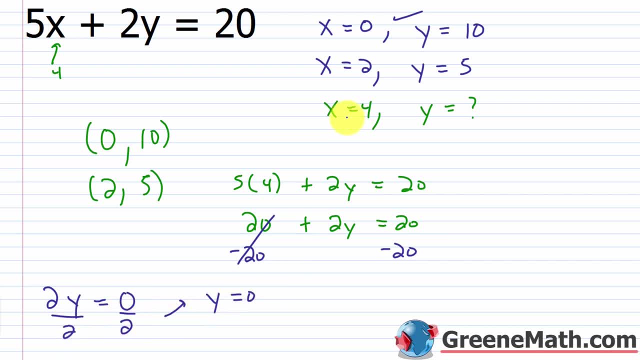 and we'll get that y is equal to 0. so if x is 4, y is 0 or, as an order, it's 4 for the x value, comma 0 for the y value. alright, so in the last lesson we talked about how to plot. 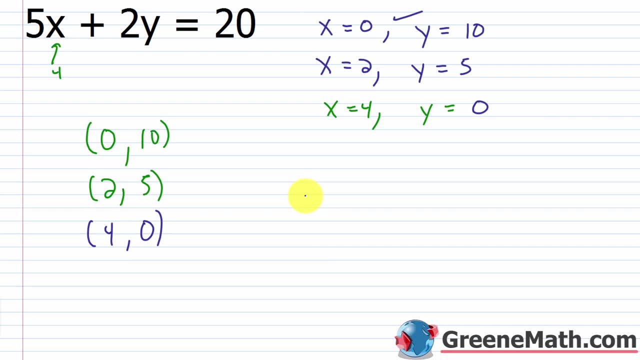 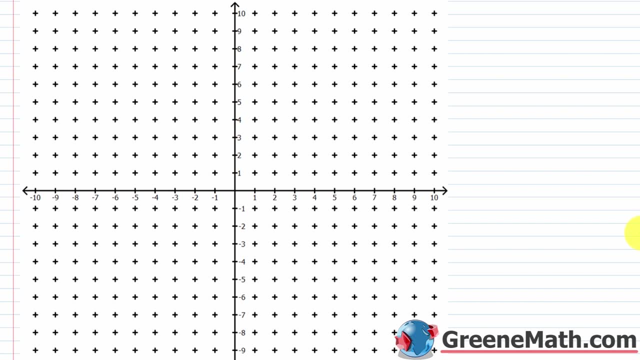 the ordered pairs. so let's go down to the coordinate plane and we're going to do that, alright, so this is our coordinate plane. and the coordinate plane consists of two number lines, so we have a horizontal number line and a vertical number line. so the horizontal number line. 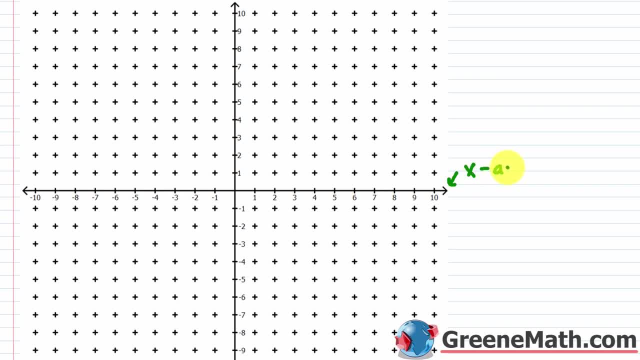 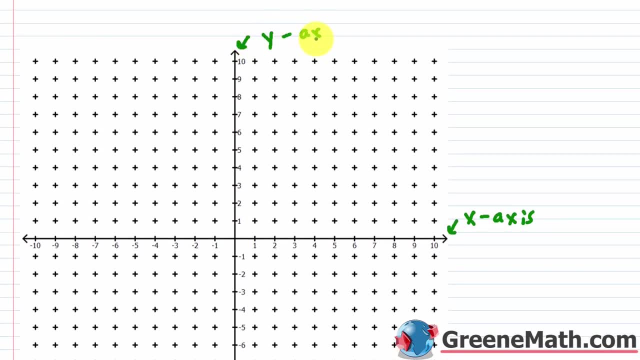 is known as the x-axis. so this is the x-axis. the vertical number line, the one that goes up and down, is known as the y-axis. so when we talk about our ordered pairs, let me paste those real quick. we have 0 comma 10, 2 comma 5 and 4 comma 0. 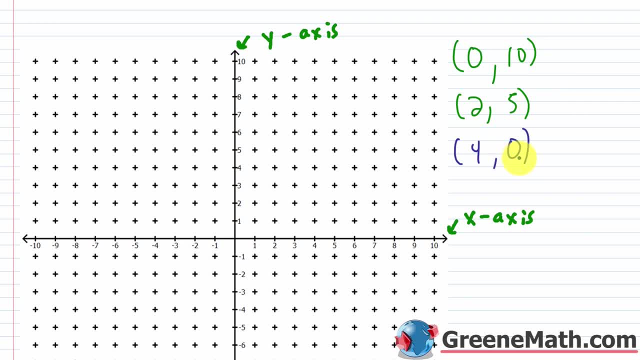 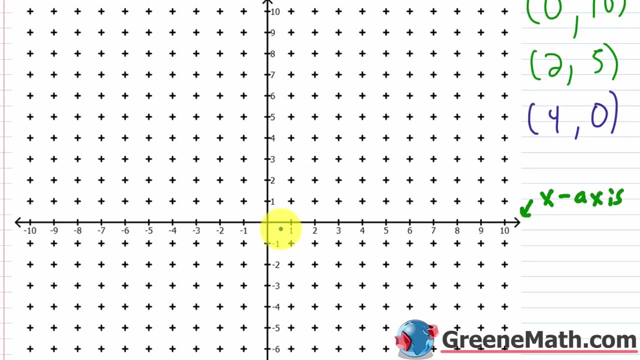 all we do is we find the intersection or the meeting point of the two locations. one location is for x, one location is for y, so in other words, for 2 comma 5, remember it's x comma y, so an x location of 2 if I go on the x-axis. 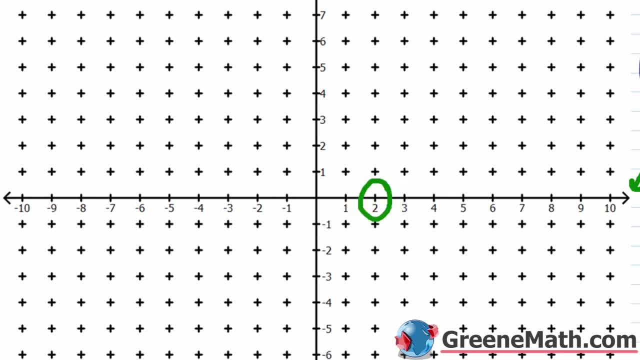 a location of 2 is just right here. for 5, the y location. I go on the y-axis. a location of 5 is right here. so where's the meeting point between the two? well, I'm going 2 units to the right, 5 units up. it's right here. 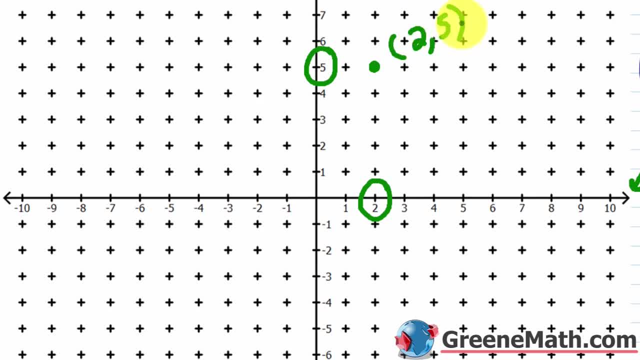 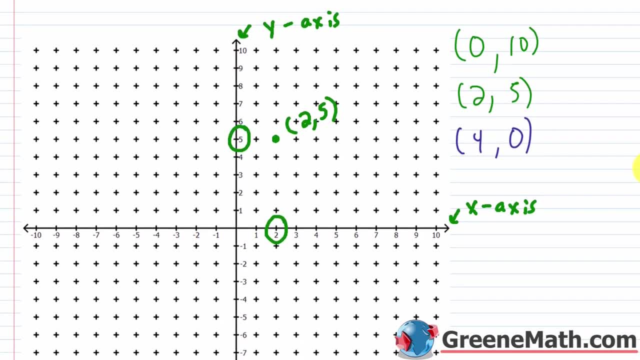 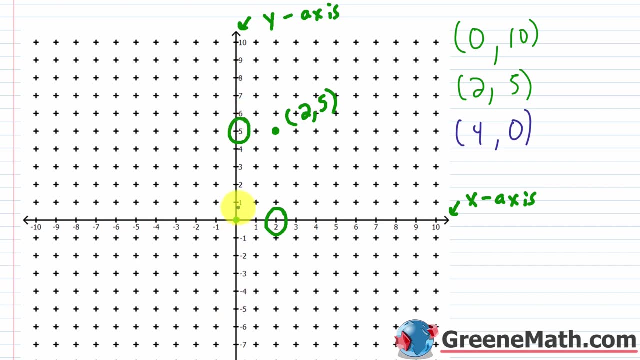 so this is the point 2 comma 5. now when we start talking about 0 as a location, it gets a little bit complex because you have to kind of think a little bit. the lines intersect at 0 comma 0. this is the meeting point. 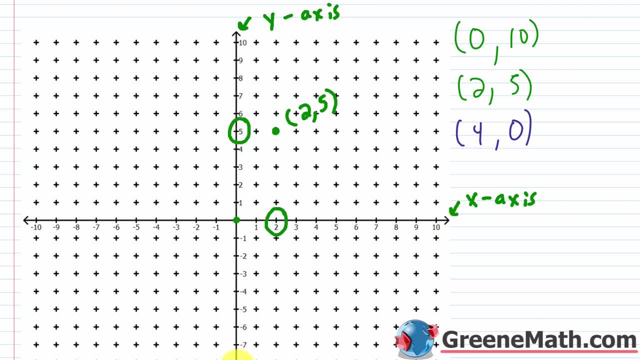 of the x-axis and the y-axis. so if I look at 0 comma 10, ok, that's telling me that I don't want to move at all on the x-axis. so I would just sit right here and I would say: well, the y location is. 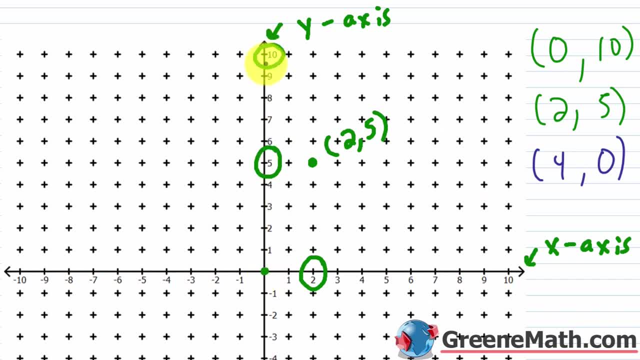 10. that's here, so I'm only going to go up 10 units to arrive at my point. this is 0 comma 10. now for 4 comma 0. now I'm going to be on the x-axis, because 4 is on the x-axis. 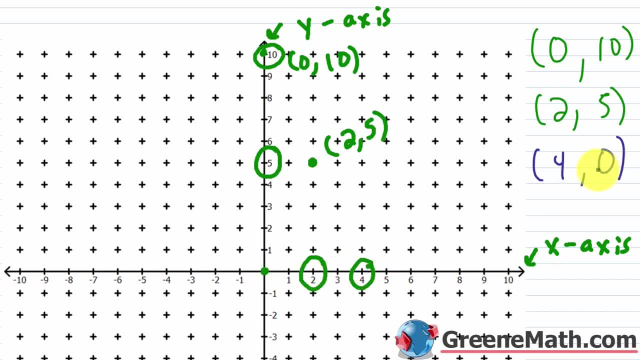 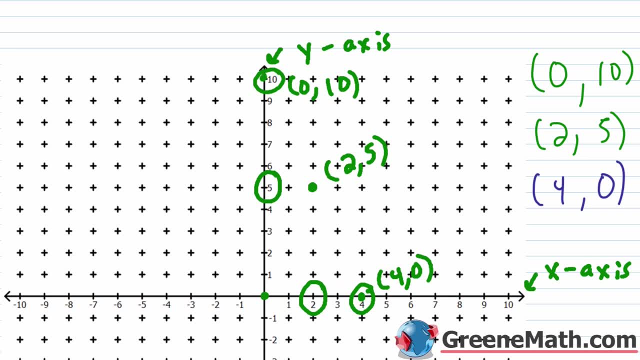 it's 4 units to the right. the y location is 0, so I'm not going to move up or down at all, I'm just going to stay on the x-axis. this right here is 4 comma 0. now once I have 2 points. 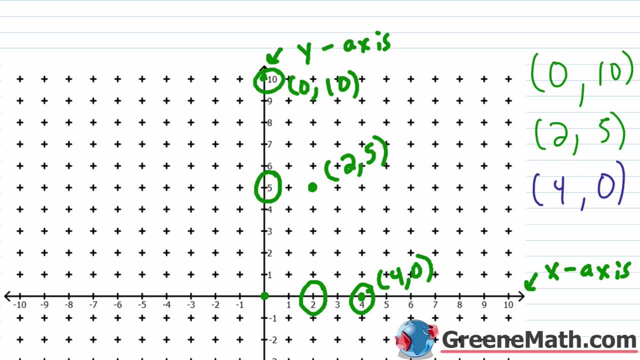 I have enough for a line. the rule is: 2 points make a line, but you always want to use a third one as a check, because I can make any 2 points line up, but if I have a third one that's off. so I get something that looks like this: 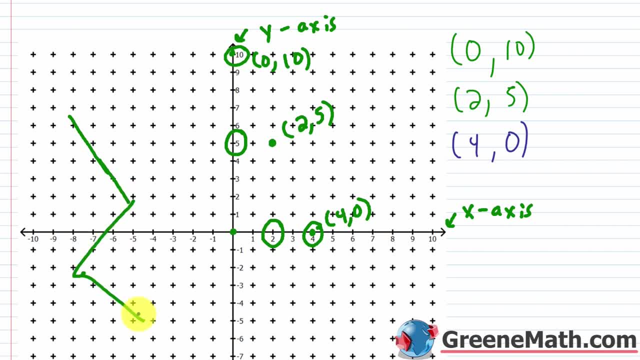 I've got a line going and then there's a point over here, so that's not a line. so you know you made a mistake somewhere. but if you have 3 points and it just kind of flows into a line, you know you got the right answer. 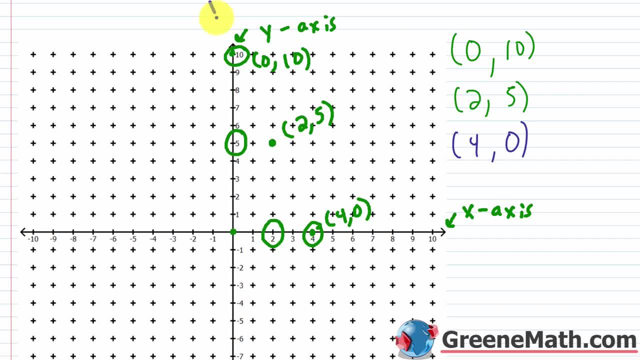 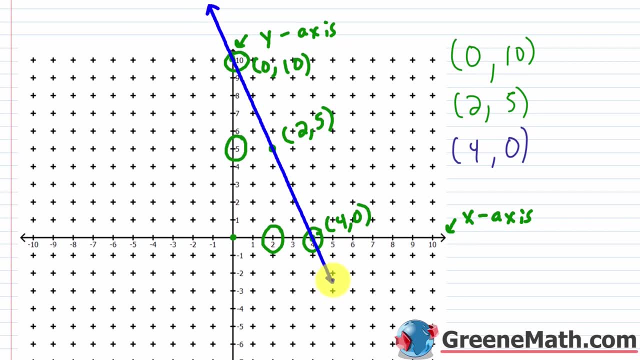 so what I'm going to do is I'm going to draw a line through our 3 points here, and what we want to do is we want to put an arrow at each end. and what does that arrow indicate? it indicates that this line continues forever and ever and ever in each direction. 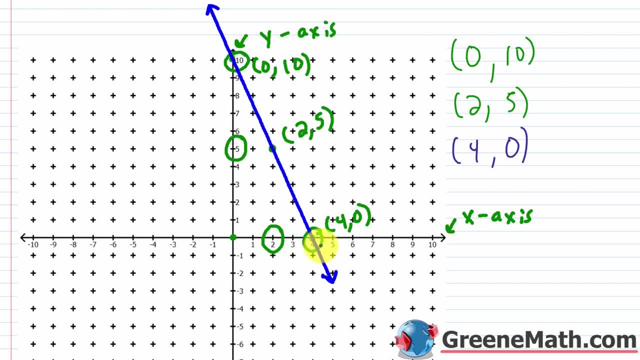 again, there's an infinite number of solutions, an infinite number of x-y pairs that satisfy this equation. every single point on this line, every single spot represents a solution to that equation that we started with, which was 5x plus 2y equals 20, and a common thing to do would just be: 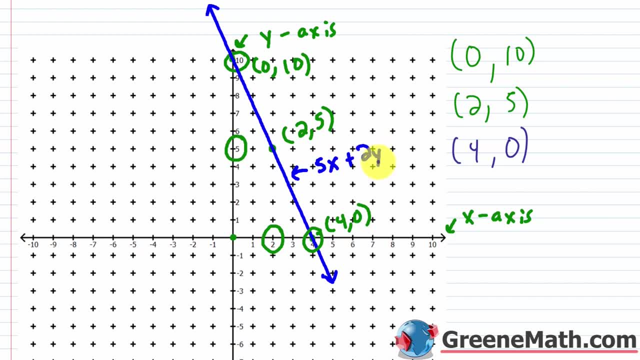 to label the line. so 5x plus 2y equals 20. this line again represents the solutions to this equation. now there's a very important concept that I want to cover with you real quick. the concept would be that of an x-intercept and a y-intercept. 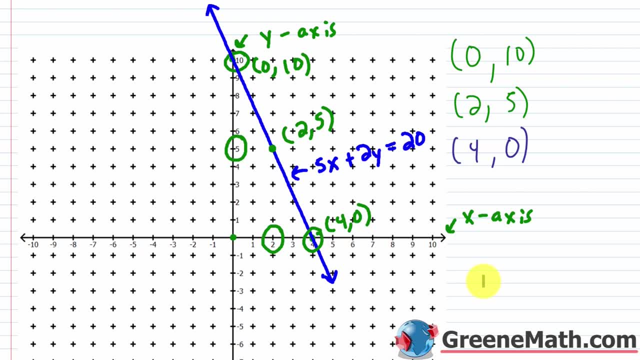 so an x-intercept is where your graph crosses the x-axis. so this right here is your x-axis. this graph crosses the x-axis right here at this ordered pair 4 comma 0. so that's my x-intercept. let me just label that real quick for you. 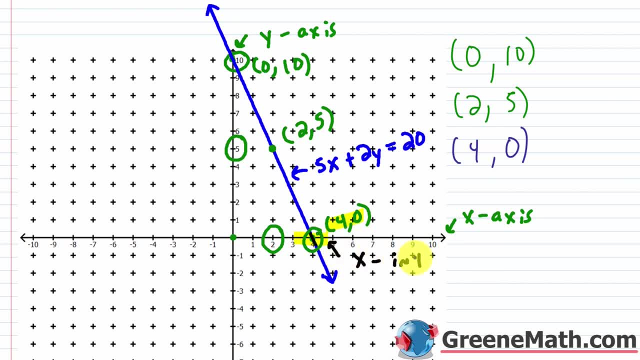 so this point, right here, is the x-intercept. now, similarly, the point where the graph crosses the y-axis- this is the y-axis going up and down- is known as the y-intercept. so this- let me just label that- right there is the y-intercept. 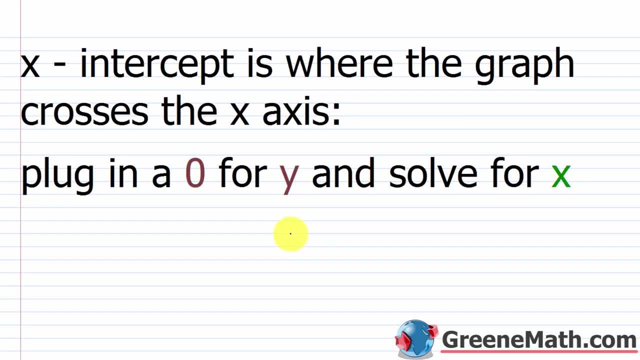 so a couple of key things here that we want to cover. the x-intercept again is where the graph crosses the x-axis. so to find this mathematically- you're not always going to be graphing stuff- you want to plug in a 0 for y. 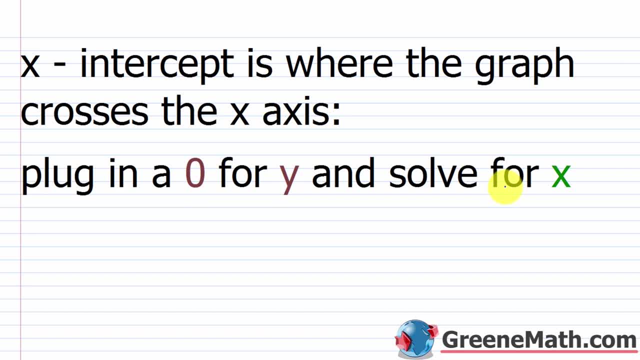 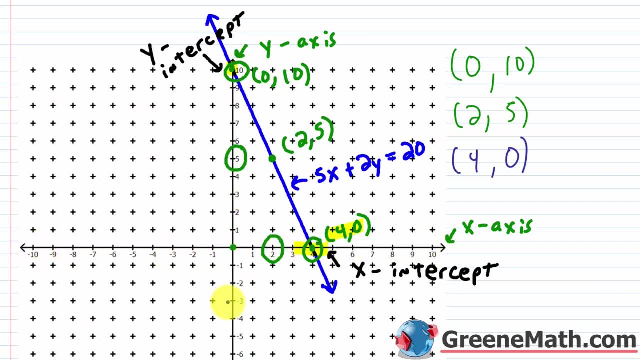 and solve for x. let's think about this for a second. let's go back to the graph. why does that make sense? where would I cross the x-axis at well, on the y-axis I can't go up or down if I'm going to hit the x-axis. 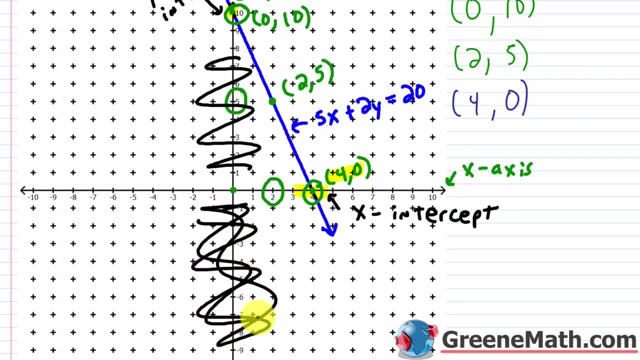 just think about erasing this axis for a minute. if I'm touching the x-axis, I've got to be at 0 on the y-axis, if I cross here at this point, I'm at 0. if I cross here at this point, I'm at 0. 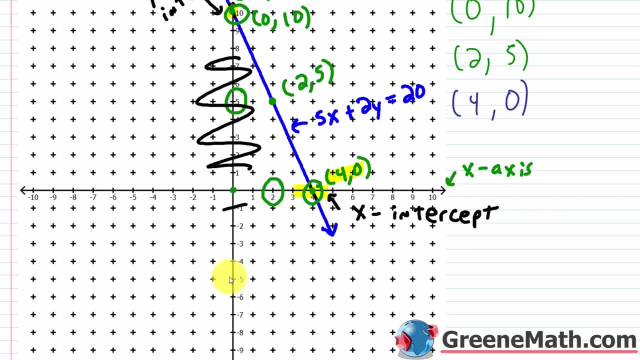 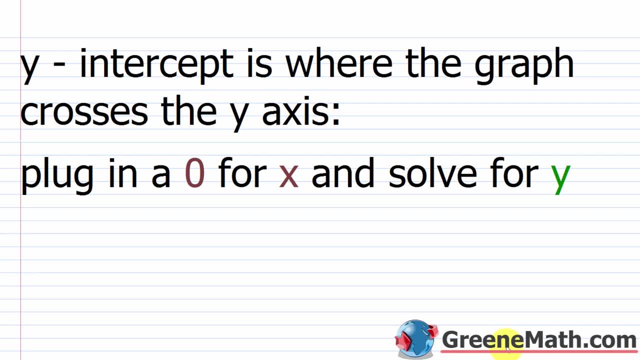 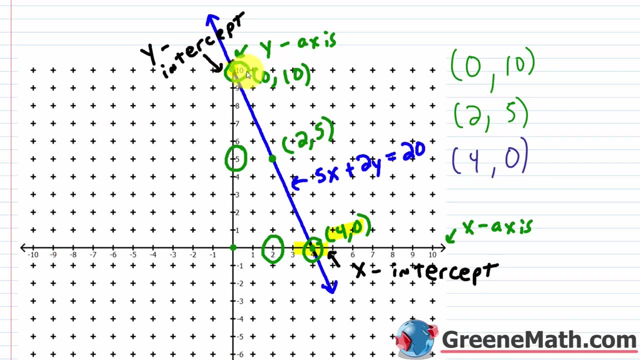 anywhere you cross the x-axis, y will be 0. so that's very important to understand. the second thing would be for the y-intercept, again, where the graph crosses the y-axis, you'd plug in a 0 for x and solve for y again. looking at this thing, we see that 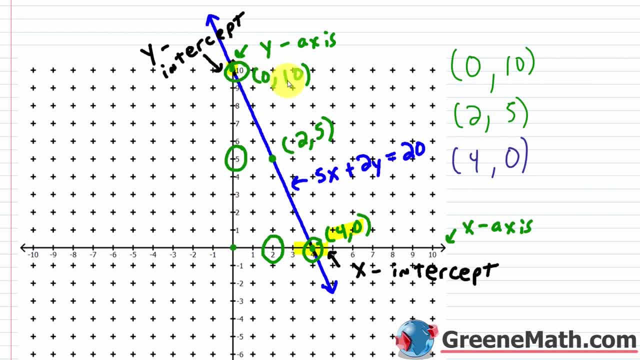 at the y-intercept, the x-location is 0. you can even see it right there: x-location of 0. at the x-intercept, the y-location is 0. so that's how we find these things. if I want the x-intercept plug in a 0 for y. 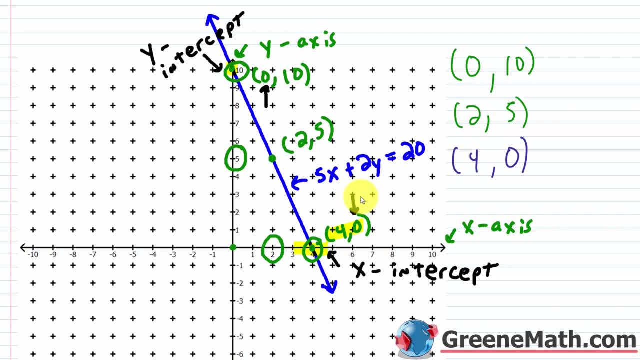 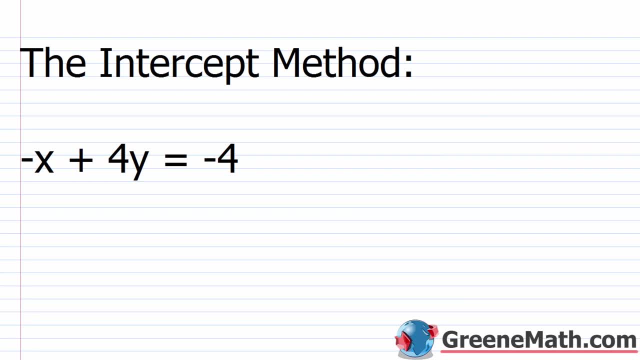 solve for x. if I want the y-intercept plug in a 0 for x, solve for y. so now that we've graphed our first equation, let's talk about one particular method to graph equations. now we just used it. it's something known as the intercept method. 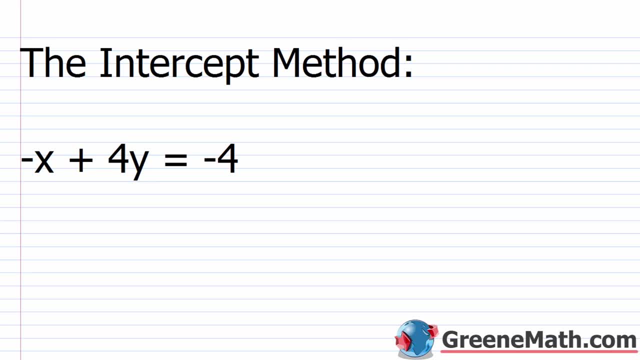 so it's easy to work with 0 as kind of one of your values. 0 is easy to work with you. multiply by 0, it disappears. you add 0, you get the same thing, so on and so forth. so the whole thing with the intercept method is: 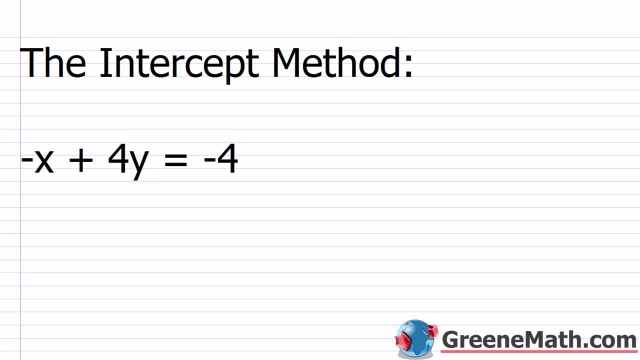 I'm going to find the x and y intercepts and then I'm going to find one point as a check. now for this one, I have negative x plus 4y equals negative 4. so when I look at ordered pairs, I create a table of values. 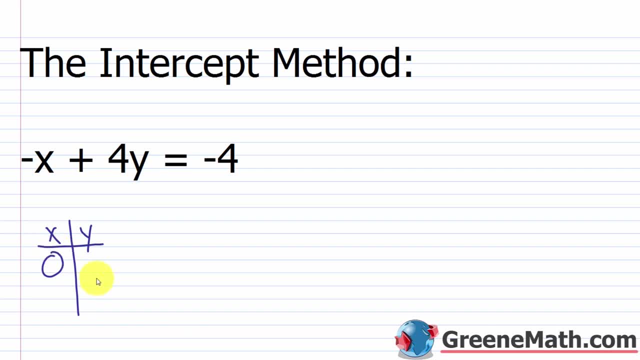 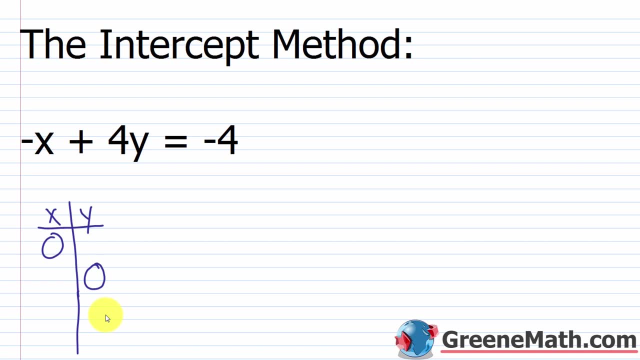 then I would find the y-intercept by plugging in a 0 for x, I'd find the x-intercept by plugging in a 0 for y, and then I'd pick some number arbitrarily to get a check. now, when you pick a number arbitrarily, 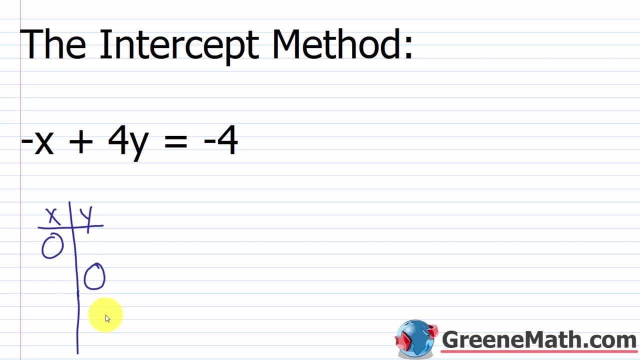 you want to make sure that you end up with integers. the reason for that is: you don't want to end up with decimals or fractions and trying to graph this on something where it still isn't integers. you can do it, but it's very, very tedious. so try to work with integers. 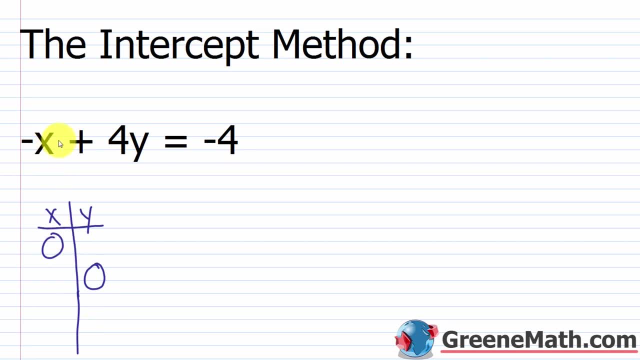 just try your best. so I'm going to start by plugging in a 0 for x. here I would have negative 0. that's just going to go away. plus 4y equals negative 4. divide both sides by 4, you get y equals negative 1. 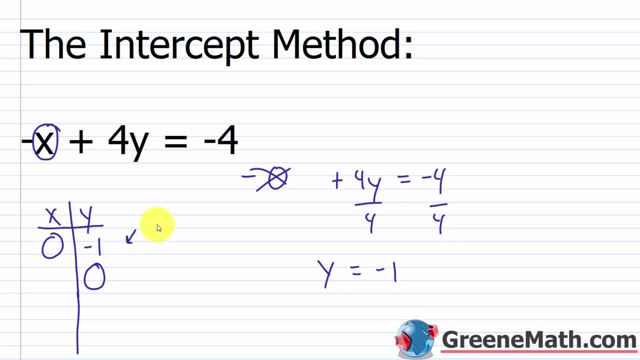 so if x is 0, y is negative, 1 again. this is the y-intercept when we graph it. I'll show you the axis there. for the other one. let's erase this real quick. we're going to plug in a 0 for y now. 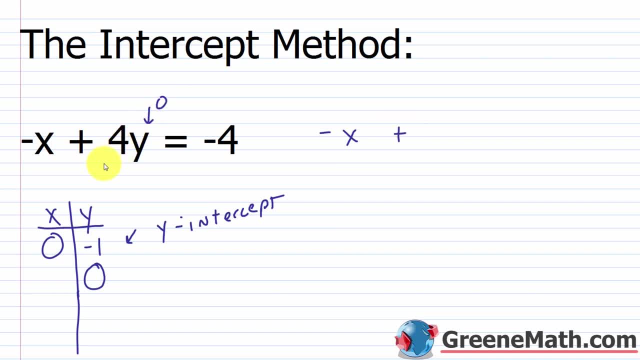 find the x-intercept, so we'd have negative x plus 0 times. anything is 0, so I can just mark this out: I can have negative x equals negative 4. multiply both sides by negative 1, I get x equals 4. so then this right here would be our. 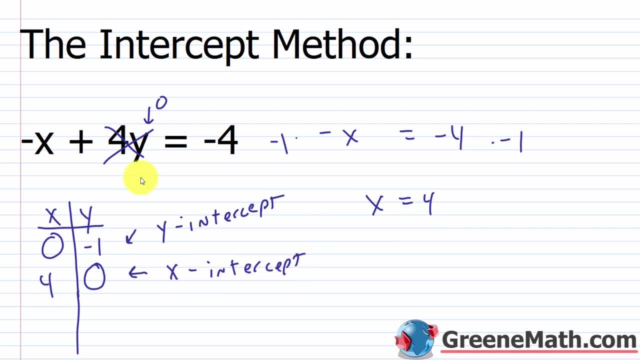 x-intercept. alright, let's erase everything. two points make a line. so if you're 100% confident that you got the right answer here, stop and do it. you can plot 0 comma negative, 1, 4 comma 0, draw a line through it. 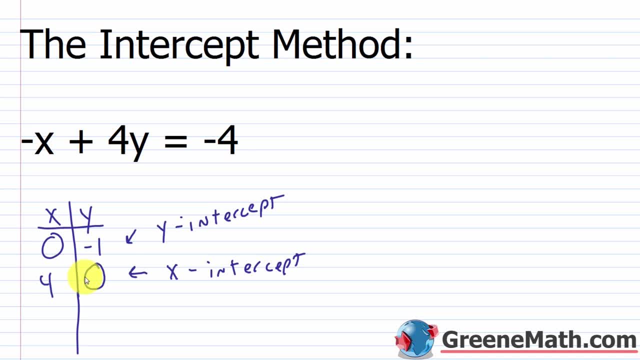 and you're done. but again, if you're like me and you're cautious, you want a third point as a check, so you want to pick something that's going to produce an integer result. so how do you do that? well, you can kind of eyeball this. 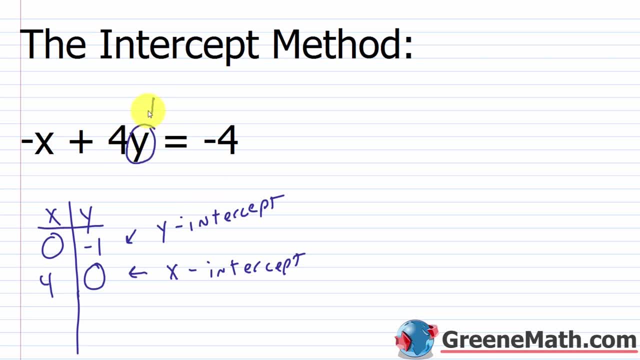 and tell what would work and what wouldn't. if I plugged in a 1 here, just think about this for a second. you would get 4 times 1, which is 4, so you'd have negative x plus 4 equals negative 4, without doing anything else. 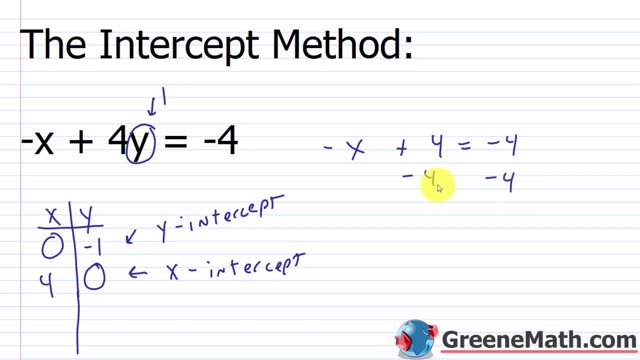 you know that's going to work because if I subtract 4 away from each side, I would have negative x is equal to negative 8. I'm going to end up with an integer result, so I'm going to go with y equals 1 and then x. 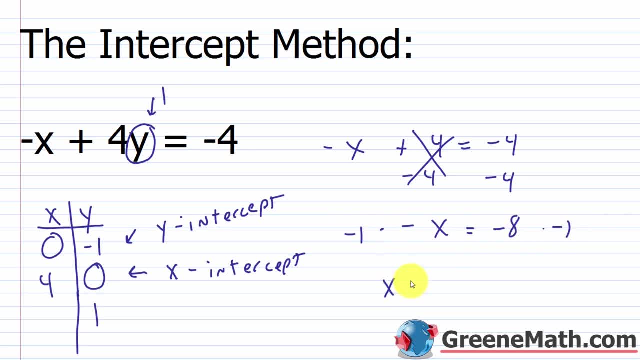 if I multiply each side by negative 1, here x is going to give me positive 8, so now I can just label this as a check. this is my check point. alright, so let's erase everything. and we have three ordered pairs. we have 0 comma negative 1. 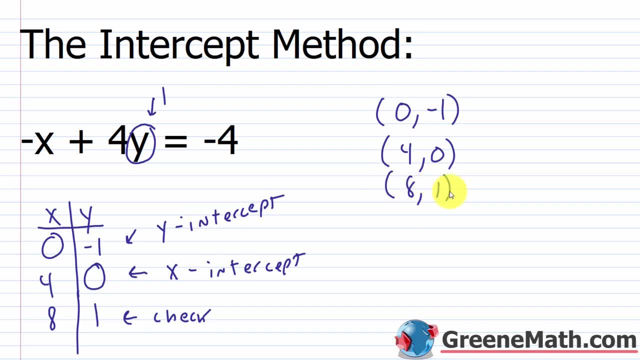 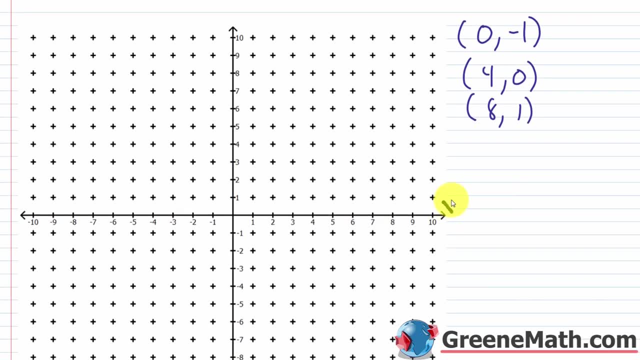 we have 4 comma 0 and we have 8 comma 1, so let's copy these. alright? so we paste our ordered pairs and again, I just want to label this as the x axis and this as the y axis, and we're going to plot each ordered pair. 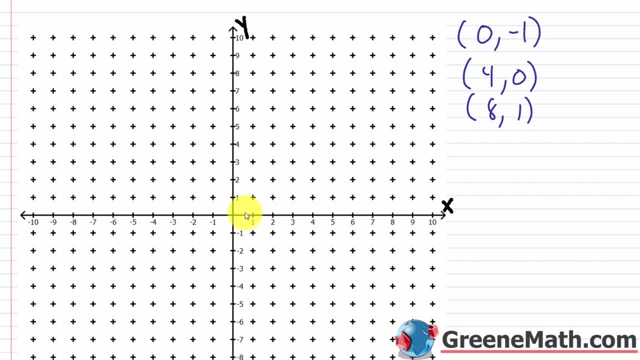 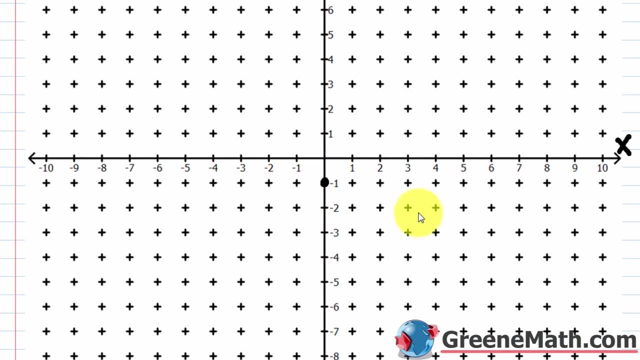 so 0 comma negative 1. so 0 is the x value, so I'm not going to move it all left or right. negative 1 is the y value, so I'm just going to move down. that's right here. now, remember, if x is 0 and y is negative 1. 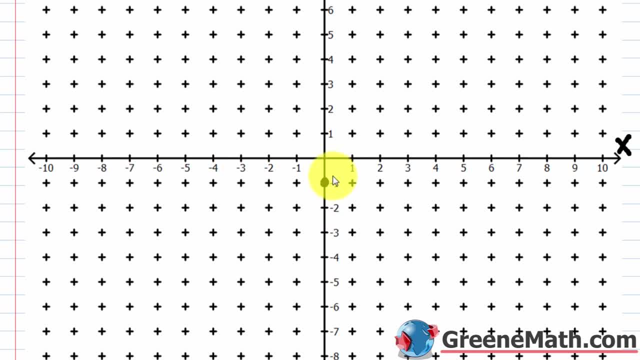 that is the y intercept, and notice how, when we graph this, it's going to cross right there, it's going to touch the y axis and again, that's the definition of the y intercept: it's where it crosses the y axis. now, the next one is 4 comma 0. 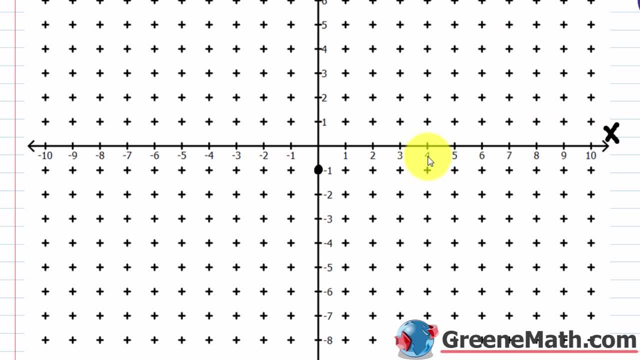 so my x location is 4, my y location is 0, so I'm not going to move it all vertically. so that's going to be right here now. notice that this is where the graph is going to cross the x axis. again, this is the x intercept. 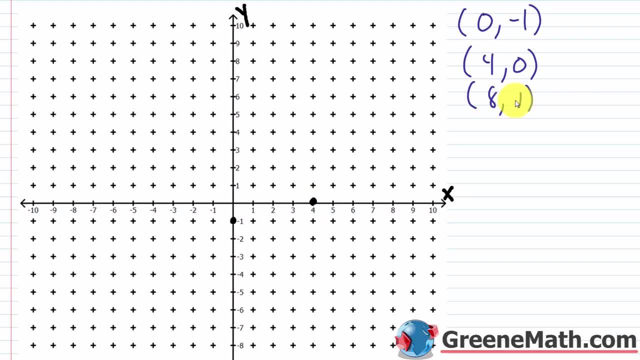 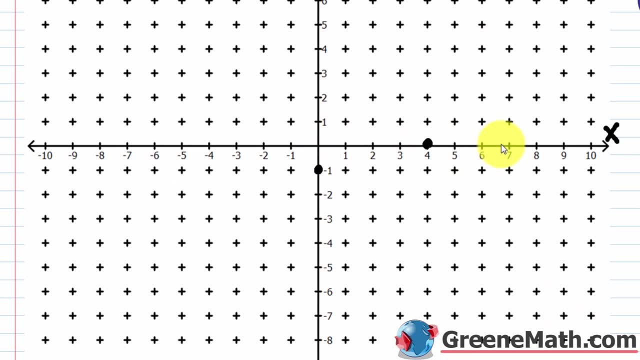 then, lastly, my point for a check is 8 comma 1. so I find 8 on the x axis. that's right. here I find 1 on the y axis. so think about it as going 8 units to the right, 1 unit up. 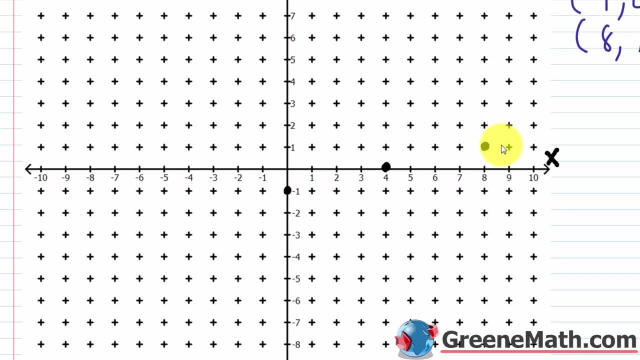 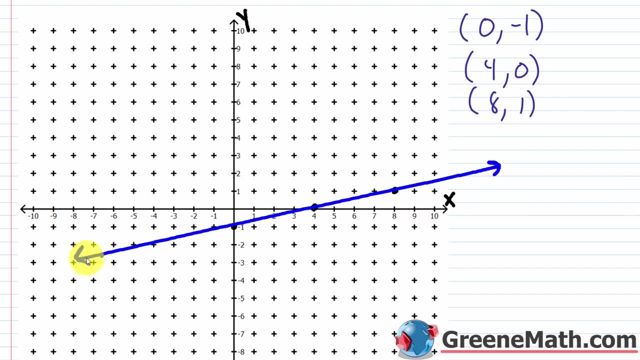 everything lines up here, so I know that I've got something going. and again I want to put arrows at each end. the arrows indicate that this line continues forever and ever and ever in each direction. so once we've graphed our line again, it's common to label it. 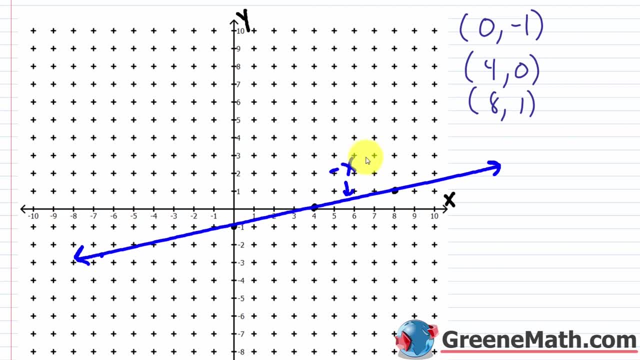 so we'll say: this is the graph for negative x plus 4y is equal to negative 4. just label it like that. you're not required to label it, but it's good practice, especially when you begin, and again I just want to call your attention to this one more time. 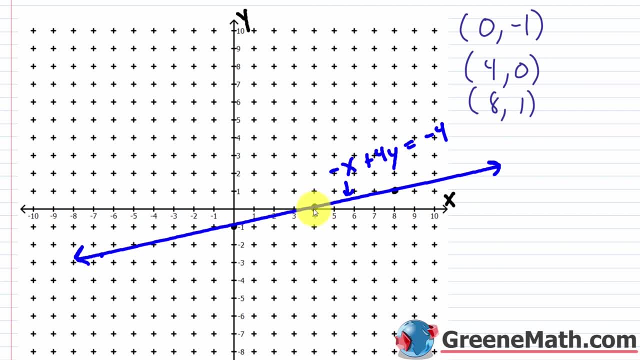 where y is 0 at the location 4 comma 0, this is the x intercept. this is where we cross the x axis. ok, where x is 0, which is 0 comma negative 1, this is the y intercept. this is where we cross that y axis. 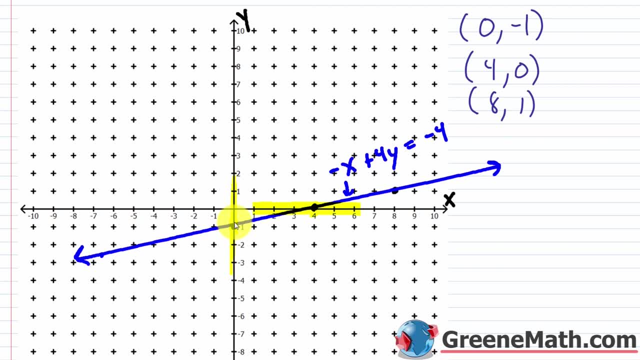 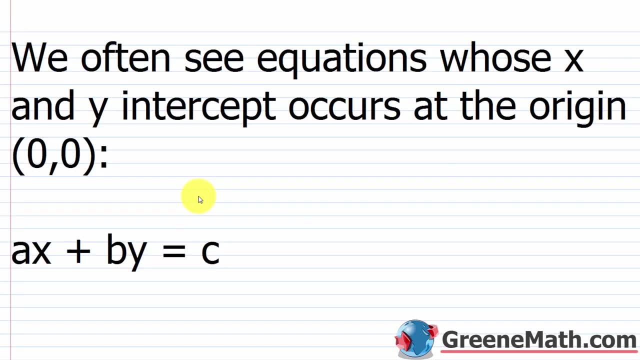 right there, ok, so again, the x intercept, the y intercept. these are very important concepts for you to get down, something you need to know right away. so kind of: the next thing that's going to occur is you're going to run across these equations where your intercept 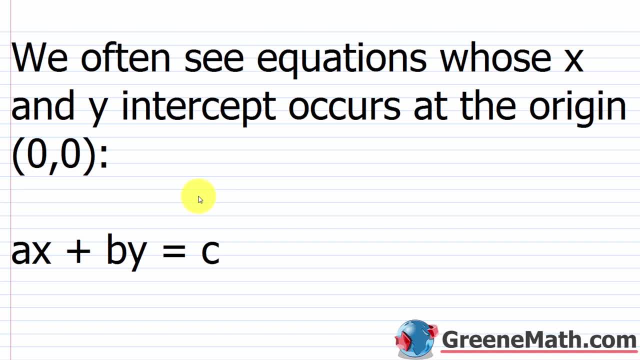 occurs at the origin. so when this occurs, the x and the y intercept are going to be there, and it's known as a line that just passes through the origin. you will encounter this as ax plus by equals c, where c is 0, so you might see something like: 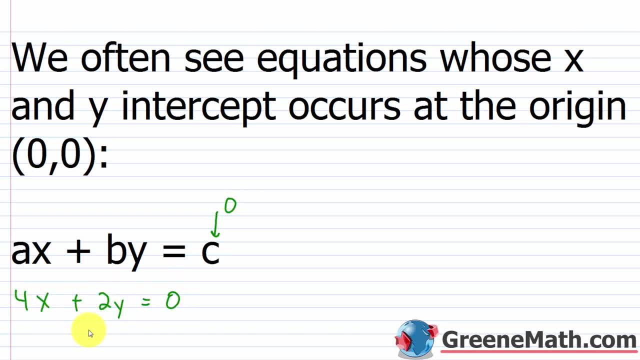 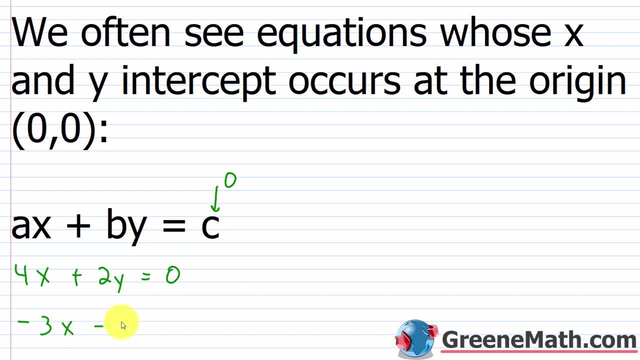 4x plus 2y equals 0. I know this is a line passing through the origin, because it's in this format- or something like negative 3x minus 7y equals 0. you're looking for something times x plus something times y. 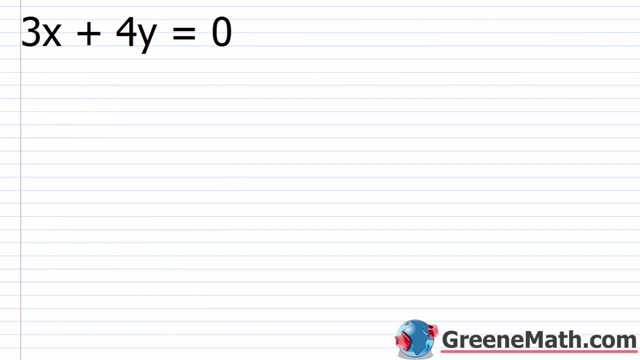 equals 0. again, that's a line that passes through the origin. so here's an example: we have 3x plus 4y equals 0. so we see it, we eyeball it, we say I know this passes through the origin. what's going to happen? 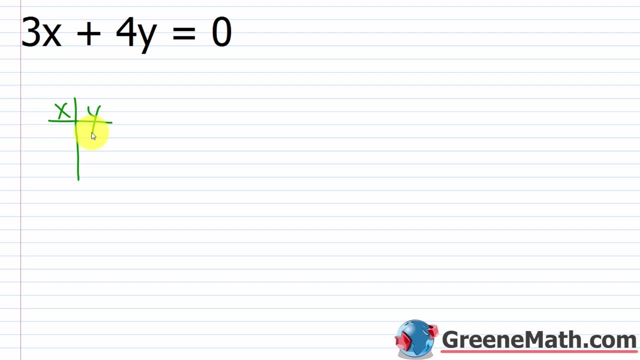 well, the x and the y intercepts occur at the same spot, so I gotta pick two additional points, not one. so if I put 0 here, I know 0 here works and you can eyeball it and see if I put a 0 here and a 0 here. 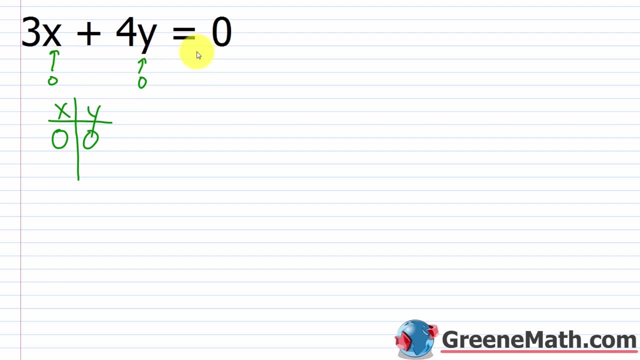 3 times 0 is 0 plus 4 times 0 is 0, 0 plus 0 is 0. so once we've identified that we get a point for free, we know automatically 0 comma 0 works again. just think about using: 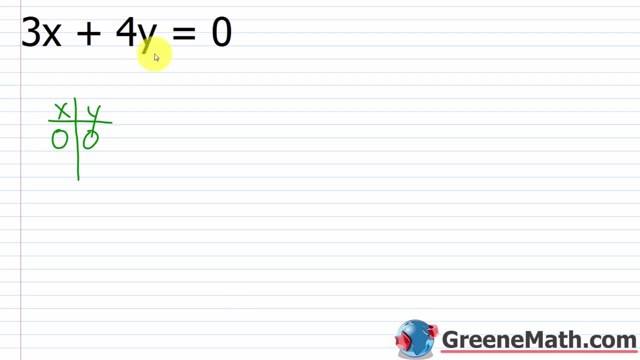 things that will produce integers. so a good way in this situation would be to subtract 4y away from each side, so I'd have: 3x is equal to negative 4y. now think about this in terms of what we could do. I know, if I multiply 3 times 4, 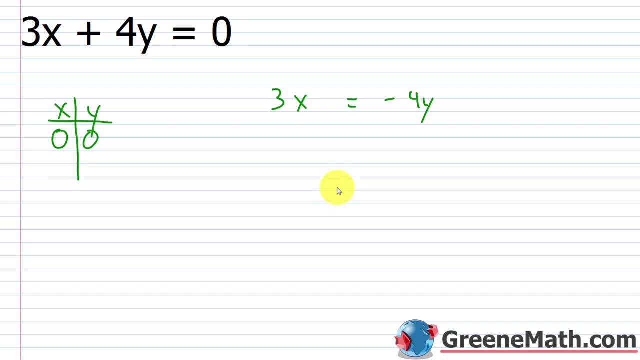 I would get something that is going to have a result, that's an integer. how do I know that? let me show you. let's put a 4 here for x and we'll continue again. a 4 there, 3 times 4 is 12. 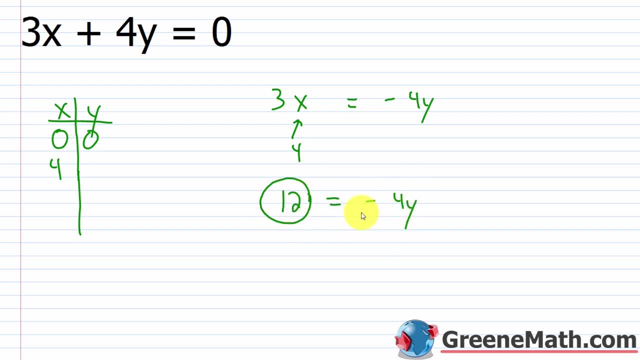 12 equals negative 4y. I know that this divided by this is going to give me an integer, because 12 is divisible by 4, so when we think about negative 4, it's divisible by that as well. so we divide both by negative 4. 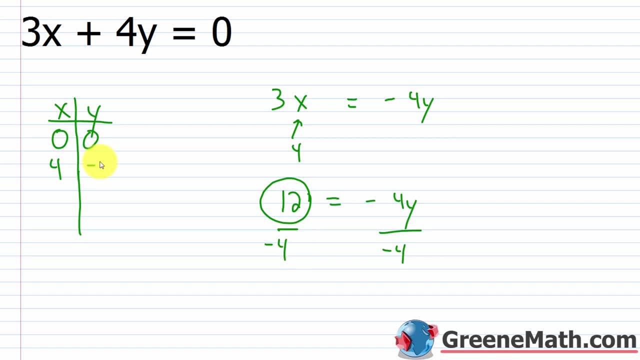 12 divided by negative 4 is negative 3. that's easy enough. now what I could do is I could switch that around. if I'm looking for an easy point, what if y was 3? well, if y was 3, I would get negative 12 over here. 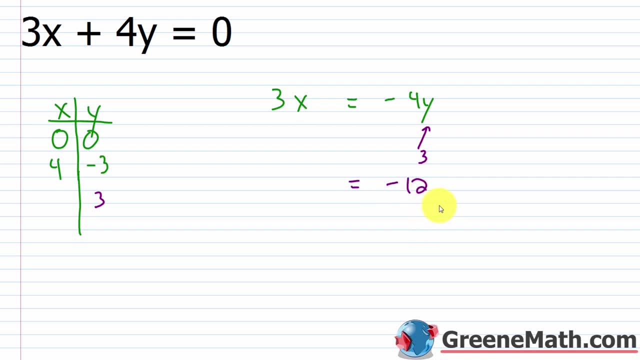 and I know negative 12 divided by 3 would give me an integer as well. so just look for little tricks like that where you can get yourself an integer, to where you're not fighting with a decimal or a fraction. so this equals 3x. divide both sides by 3. 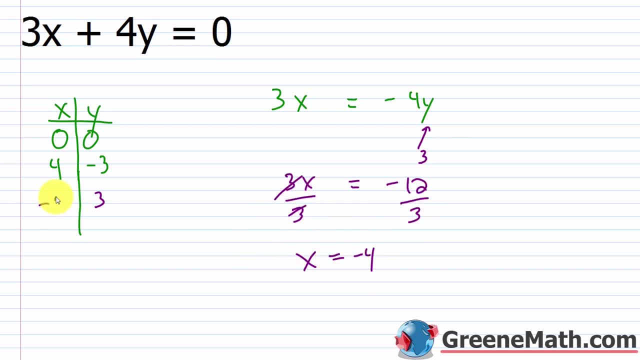 you get, x is equal to negative 4, so this is negative 4, and so we have 3 ordered pairs. we have all integers, so it's going to be easy for us to graph. so we have 0 comma 0, we have 4 comma negative 3. 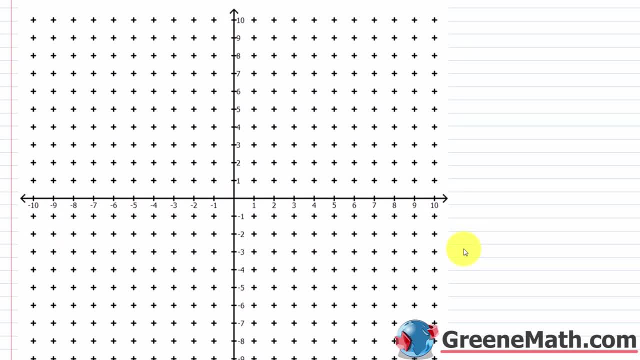 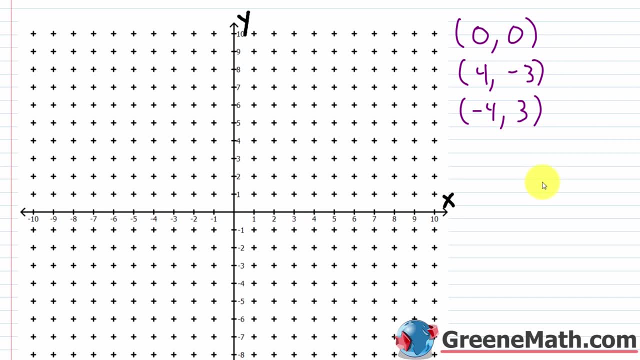 and we have negative 4 comma, positive 3. so again come down to my coordinate plane. this is x, this is y. I'll paste my ordered pairs. so the first one is 0 comma 0. so that's at the origin. that's right here now. remember we said that this was a line. 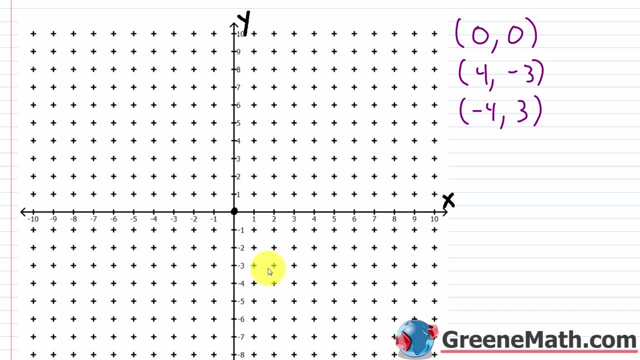 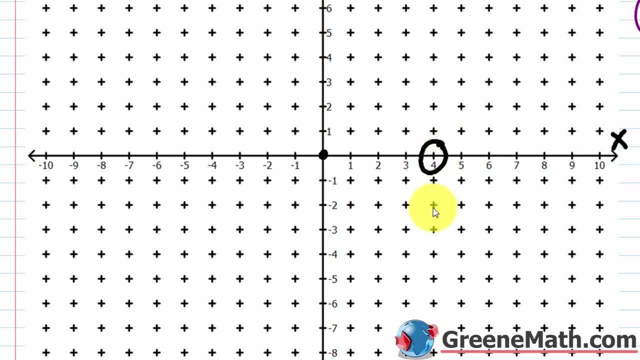 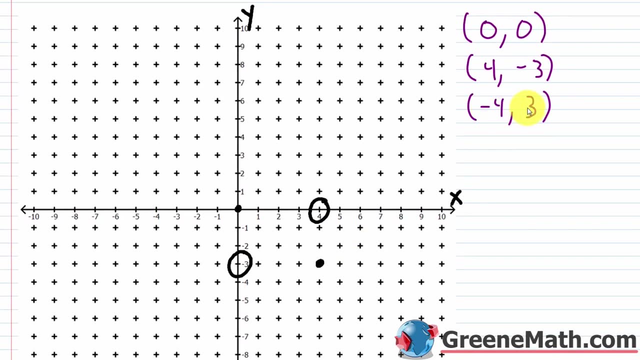 that passed through the origin. so we expect that point is 4 comma negative 3. so 4 units to the right, that's my x location. 3 units down, that's my y location 4 right, 3 down is right here. then the other one is negative, 4 comma 3. 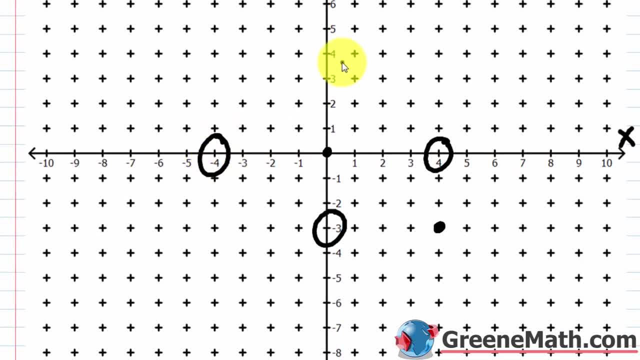 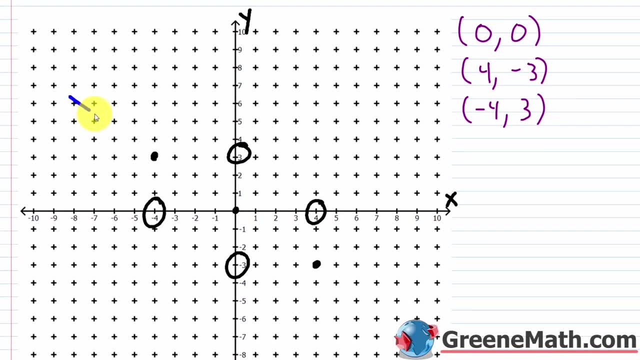 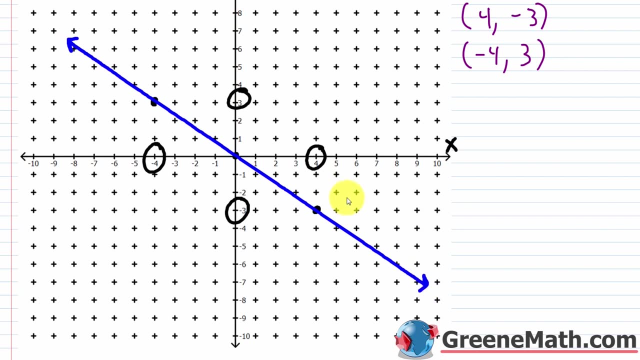 so 4 units to the left, 3 units up. so 4 left, 3 up is right here and now. we just draw a line and connect the points. ok, and again, I'm going to label this as the equation 3x plus 4y. 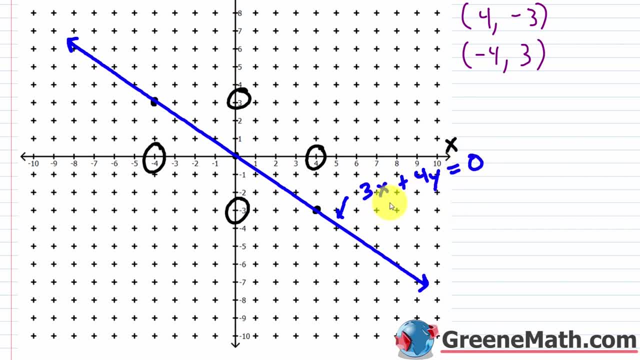 equals 0. so again you see something in this format: ax plus by equals 0. you know it passes through the origin and again you can look at that and remember that your x intercept and your y intercept occur. at that point it's passing through both of those. 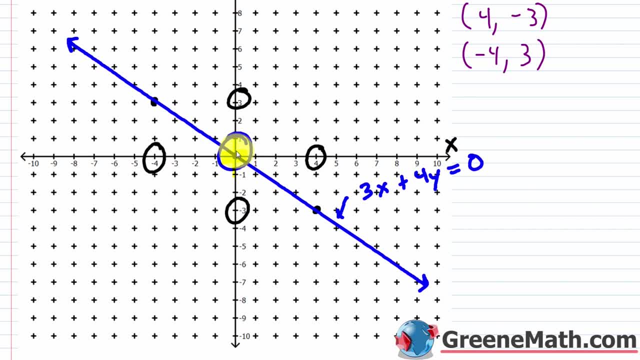 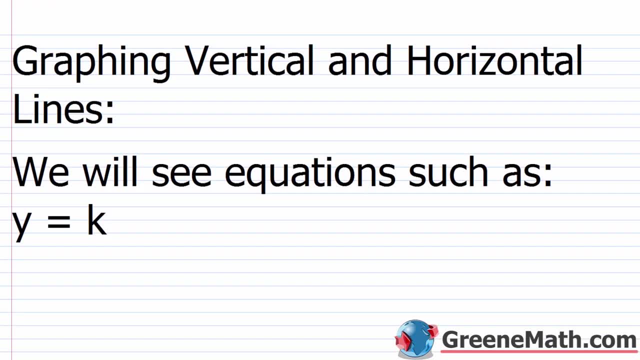 ok, it's passing through the x axis and the y axis when it hits that origin. so that's your x and your y intercept, alright. so pretty easy overall to graph a linear equation of two variables. I know that the majority of you remember this from algebra 1. 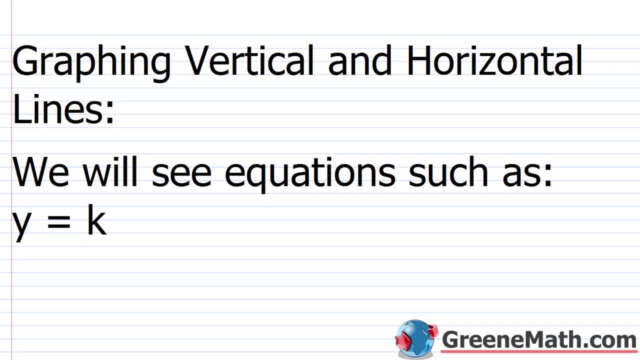 and so this is really just a review for you. but I want to cover something else before we kind of get into slope and start talking about some things in algebra 2 that we didn't talk about in algebra 1: graphing vertical and horizontal lines. this is something that students 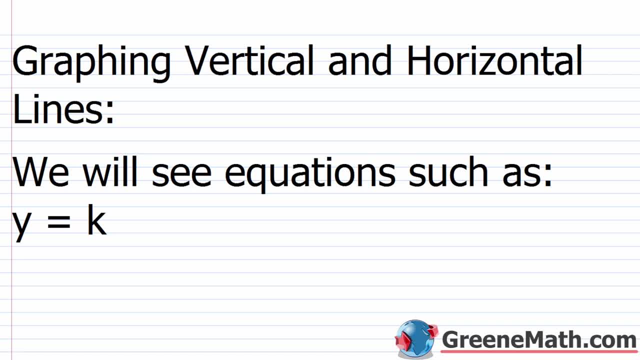 even though they took algebra 1, they still struggle with it. you will see equations such as x equals k. remember I told you the definition of a linear equation of two variables was ax plus by equals c, where ab and c were real numbers. so 0 is a real number. 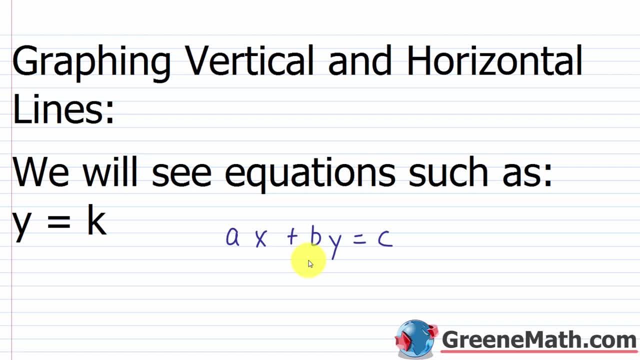 and I said that a and b cannot both be 0, but one of them could be 0. so what I have here is basically the case where this is 0, so 0 times x plus something times y, let's say it's 3y equals. 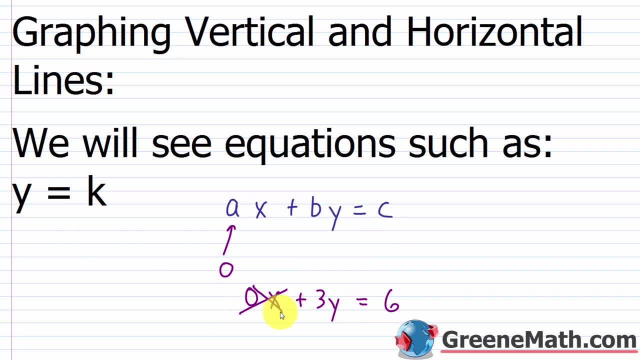 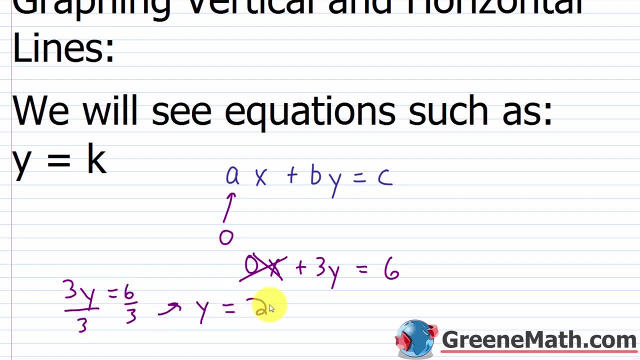 6. so 0 times x is just 0. so this is gone. I have 3y equals 6, divide both sides by 3 and I get y equals 2. so this is an equation where y always equals 2, no matter what the value is for x. 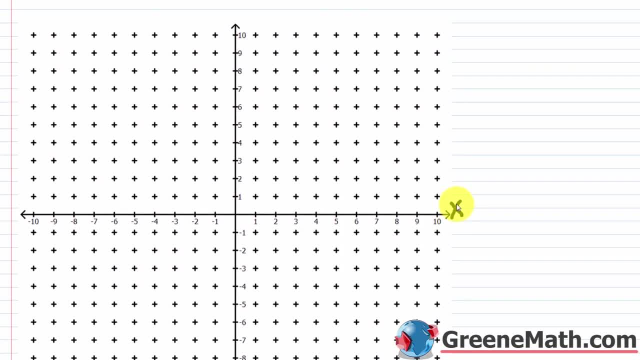 so to graph something like that again, this is your x axis. this is your y axis. if y is equal to 2- again I showed you could write this as 0x plus. in this case we've already simplified it, so let's just say: plus y equals 2. 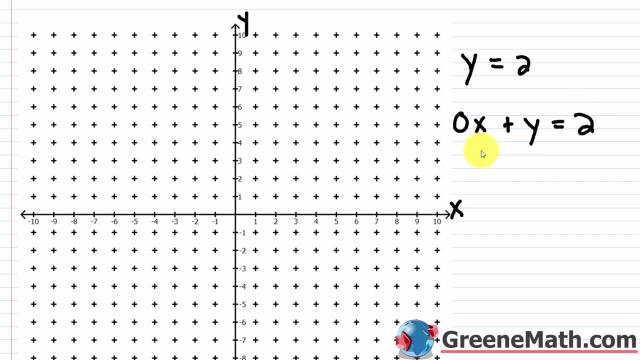 anything I plug in for x, if I was to make a table of values, will become 0. so let's say I just say, alright, here's x, here's y. let's say I choose 3 for x. well, 3 times 0 is 0. 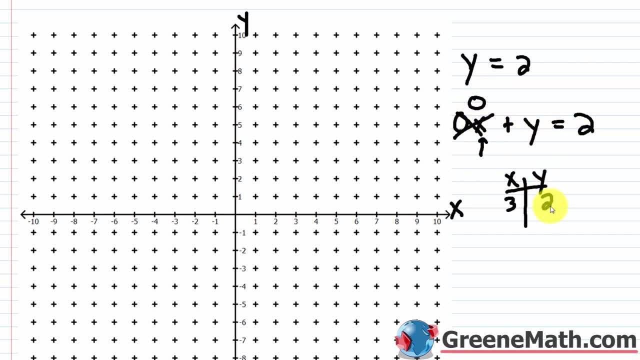 so this is going to cancel. every time it be 0, I'm just left with y equals 2. so no matter what I plug in for x, it becomes 0 and I'm left with y equals 2. so x equals 0. let's say negative 5. 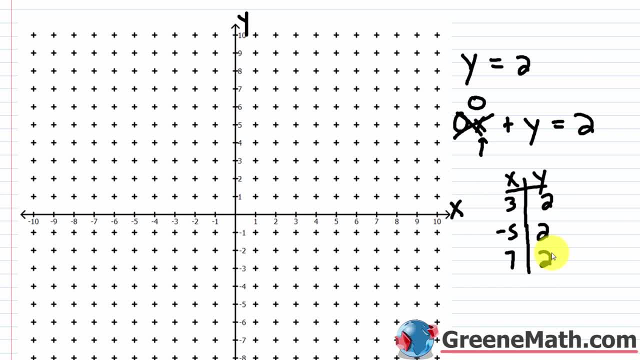 y is 2, x equals 7. y is 2, x equals 1 million. y is 2, so y just always equals 2. so what you do for something like this? you just find 2 on the y axis and you draw a horizontal line. 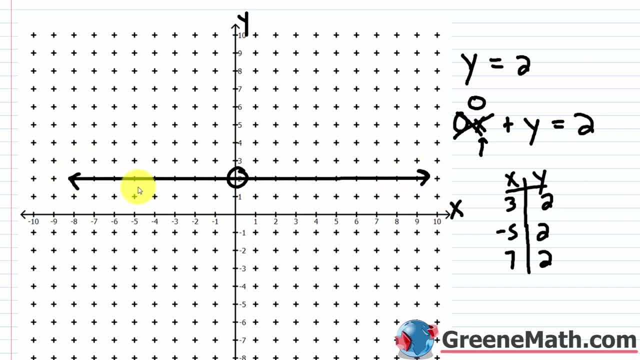 that's it. that's all you have to do. ok, and you still want arrows, because this goes infinitely in the left and the right direction. so if I gave you something like, let's say, y equals 5, now let me label this one before we move on. 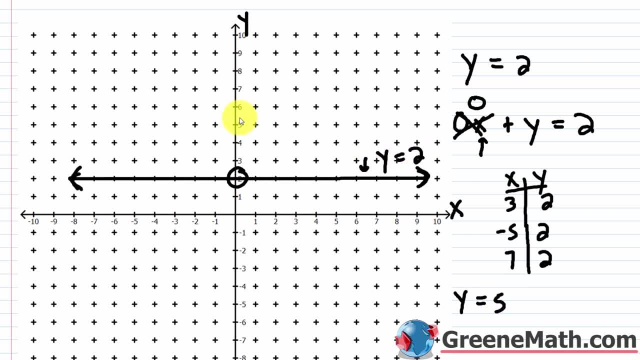 this is y equals 2. if I gave you y equals 5, you would just find 5 on the y axis. again, for any x value you choose, y is 5. so if x was negative 3, y would be 5. if x was 6. 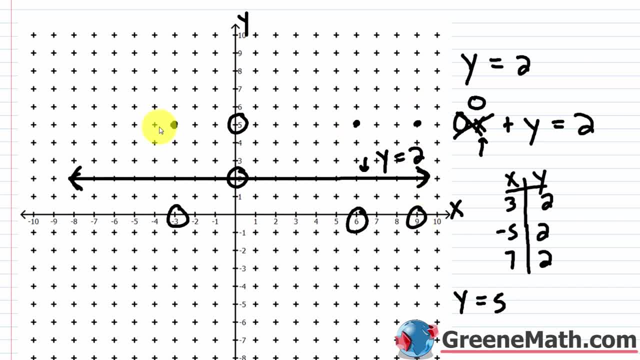 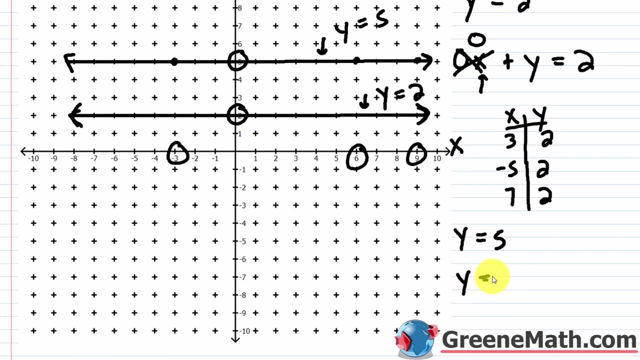 y would be 5. if x was 9, y would be 5. we would just draw a horizontal line, put our arrows and say this is y equals 5. and let's say- I saw something like y equals, I don't know, negative 7. well, I just find negative 7 on the y axis. 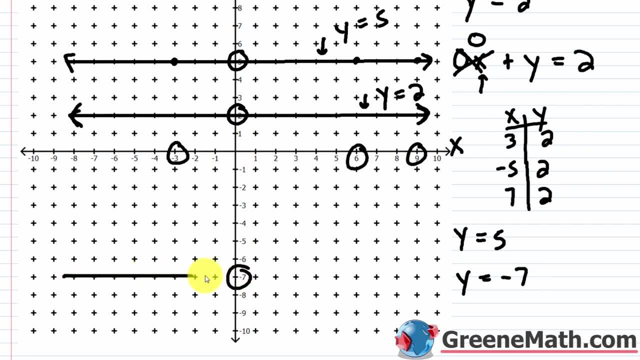 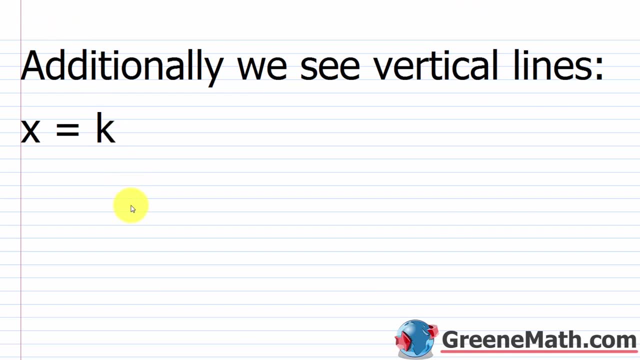 right there, draw a horizontal line. ok, it's just that simple. let me label this as y equals negative 7. alright, so additionally- the last thing we're going to talk about in this lesson- we will see vertical lines. so this is where x equals some value. so again, I go back to my 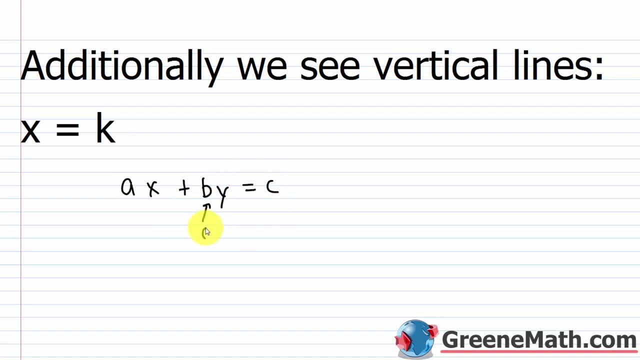 ax plus by equals c. well, in this case b is 0, so ax plus 0y equals c. for simplicity let's just say: a is 1, so we have x plus 0y equals c. 0 times anything is just 0 x equals c. 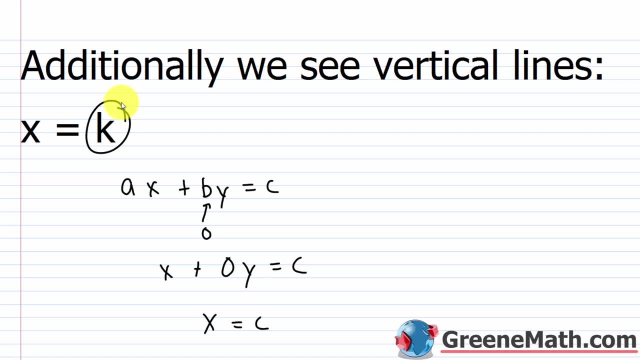 or in this case, we just put k. it just means we're representing k and c. it's just some real number. it can be anything. x could be, let's say, 4, or x could be 6, or x could be 10. whatever it is, it's just going to be a vertical line. 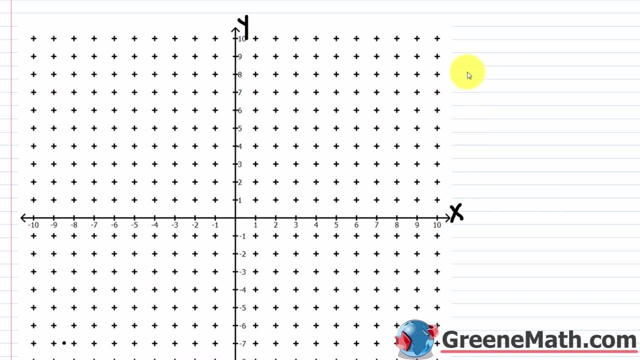 so let me show you that real quick. so let's say we had x is equal to 4. again I go back to my table of values. if I write this as x plus 0y equals 4, no matter what I plug in for y, x will equal 4. 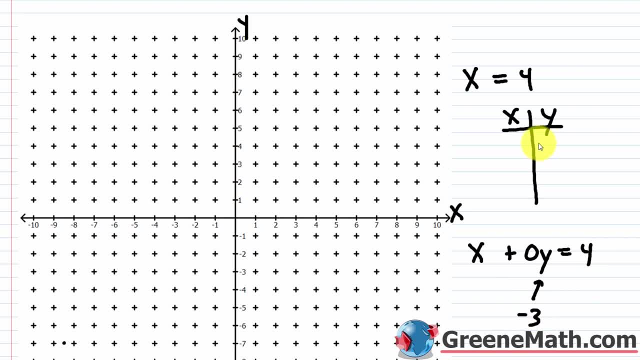 let's say I plug in negative 3, so negative 3. well, negative 3 times 0 is 0, so this cancels and becomes 0. you just have x equals 4 and that's true for anything. it doesn't matter what you plug in. 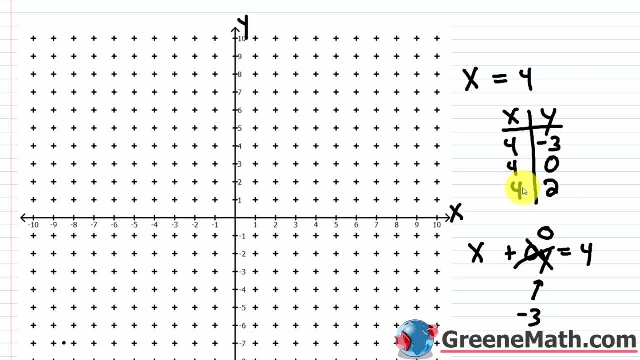 so you can pick some points. let's say negative 3,, 0, and 2, and in every case it's going to be 4 for x. so the simple way to do this is not to plot points, which is right here, and to draw a vertical line. 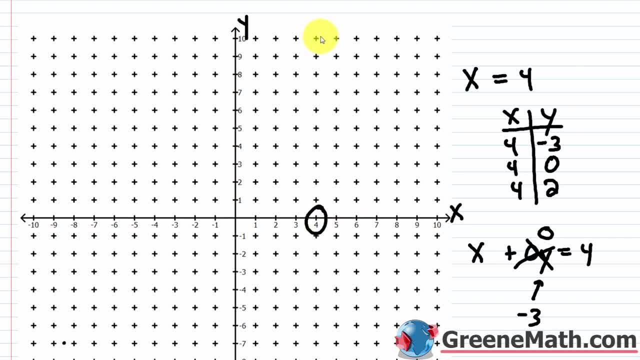 because no matter what the value is for y, so all these values for y at 10, x equals 4 at 8, x equals 4 at 5, x equals 4 at 3, x equals 4, so on and so forth. 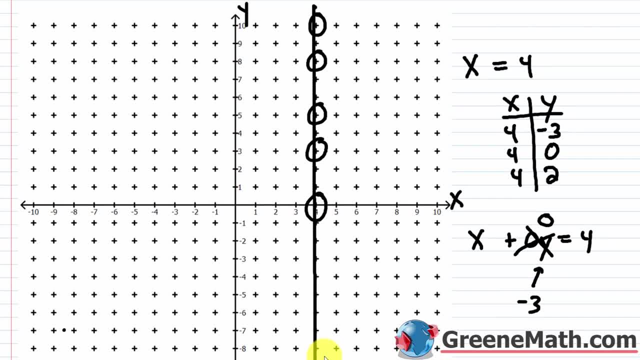 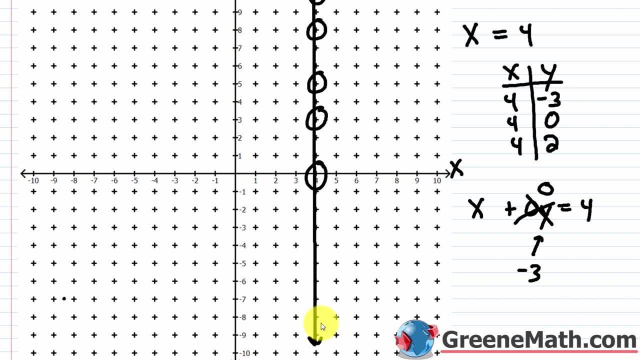 so it just becomes a vertical line and you want to make arrows at the top and the bottom just to show that continues forever and ever and ever, in both directions. alright, so let's try another one. let's say x was equal to- I don't know- negative 8, for example. 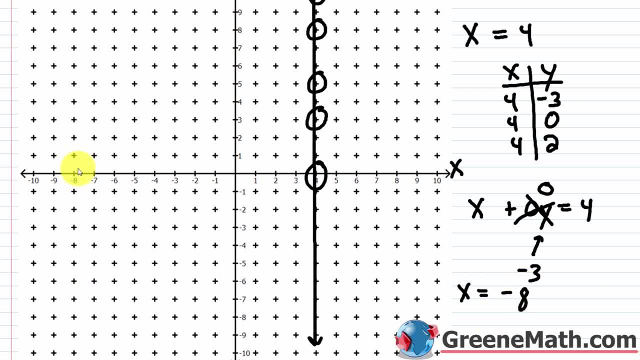 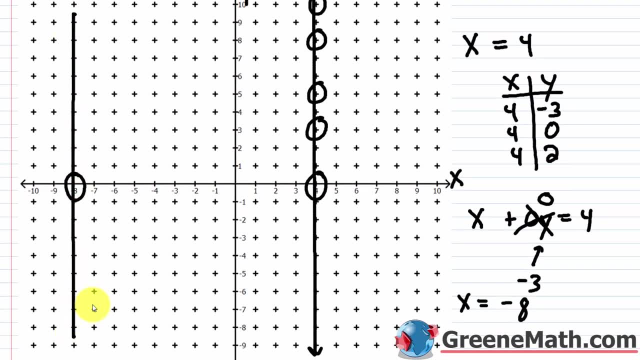 what would I do there? well, I'd find negative 8 on the x axis, which is right here, and I would simply draw a vertical line. again, make sure to use my arrows. let me label everything, make it clear. so, again, this was: x equals 4. 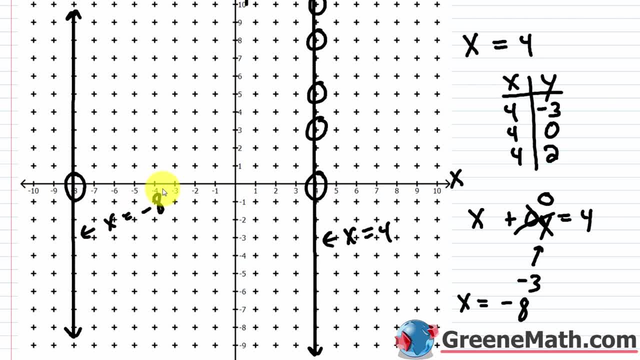 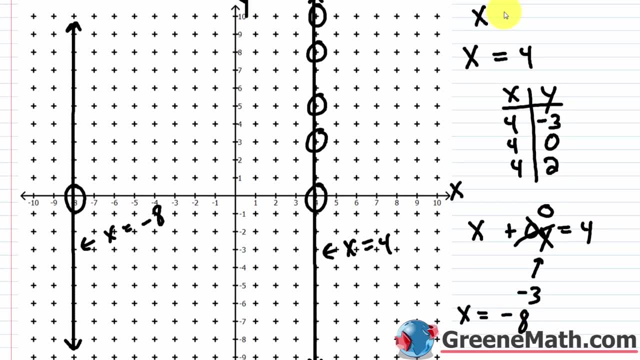 and this is: x equals negative 8. so we can look at things and say, well, x equals negative 8. so if I have x equals negative 8, I can really think about it as x plus 0 y equals negative 8. well, think about some values for y. 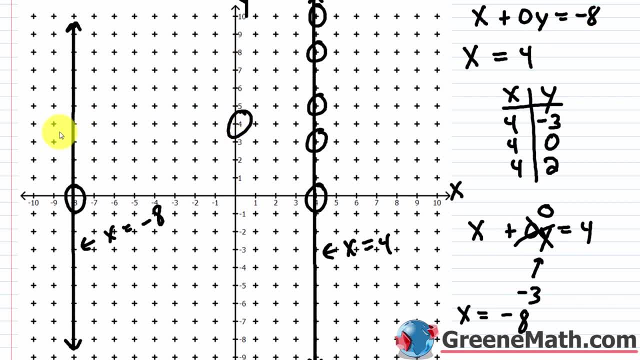 if y is 4 oh x is negative 8, so that's right here. if y is 1 oh x is negative 8, so that's right there. if y is negative 5 oh x is negative 8, that's right there. that's right there. 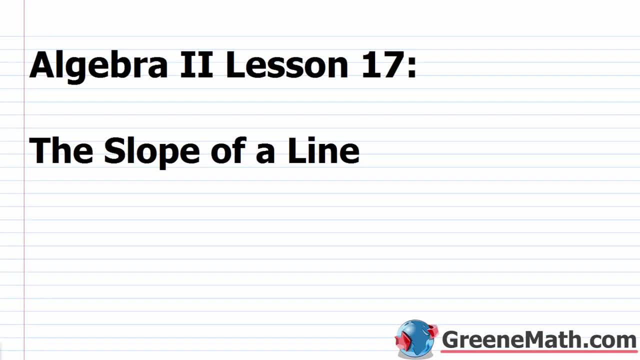 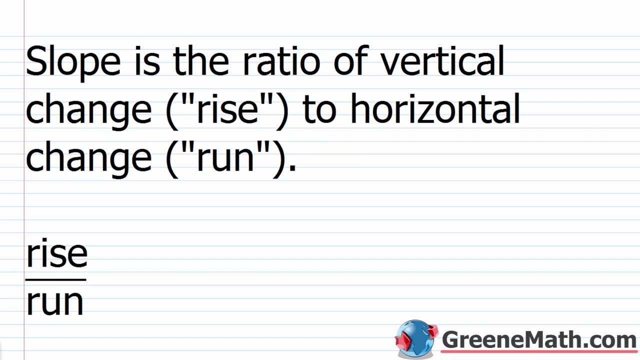 that's right there, and then we'll come back to that. so let's try again. let's try to do this again. find that number on the x axis, draw a vertical line. in this video we're going to learn about the slope of a line. so for the majority of you, 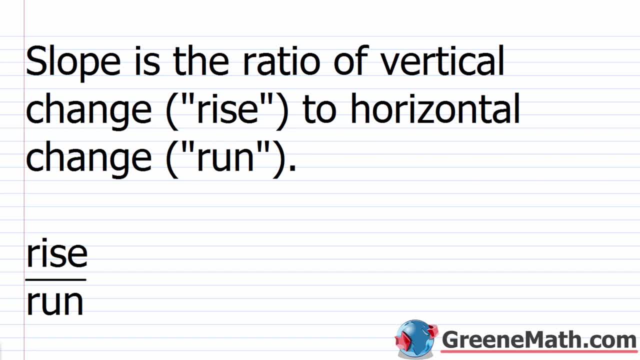 you've taken algebra one already and you're already very comfortable with the concept of finding the slope of a line. for others, you skipped. tell you if you fall into that category. you can definitely pick up slope. from just watching this video It's a very, very easy concept. So the slope of a line is nothing more than a measure. 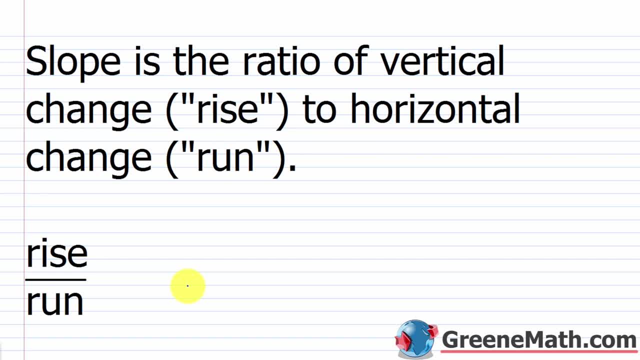 of its steepness. You can think about some real world examples of this. You can think about the slope, or the pitch, as it's called, of a roof. We all know that different roofs have different steepnesses, and so they have different slopes. You can also think about the slope of the roads. 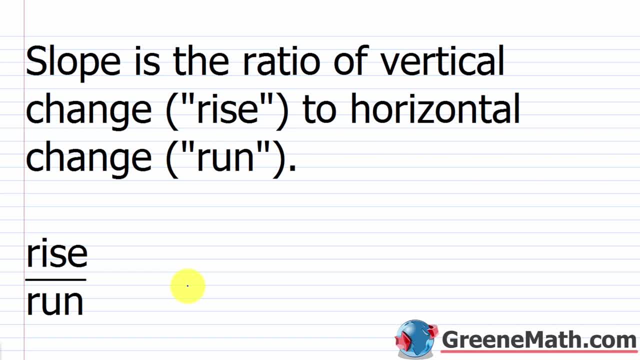 that you drive on. This is often called a grade, So different roads that you drive on, depending on where they are, are going to have different steepnesses, different slopes or different grades. So slope is nothing more than the ratio of vertical change, which is known as the rise. 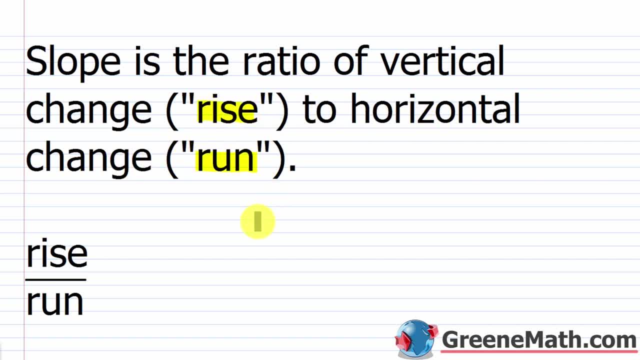 to horizontal change, which is known as the run. So we're going to hear this for the rest of our life: Slope is the rise over the run. I want you to write that on a flashcard and memorize that. You're going to hear it over and over and over again, So you've got to kind of know that. 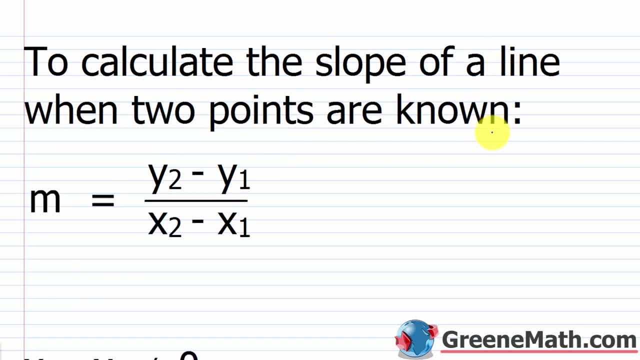 All right. so actually calculating slope is very, very easy. We're given this formula for when we know two points on the line. So to calculate the slope of a line when two points are known, we're given this formula again. that's known as the slope formula. So M stands. 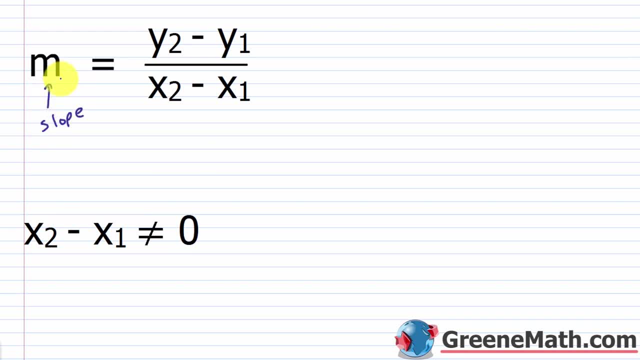 for slope. That's another thing you want to write down, because a lot of times you're expected to notate your slope with M. So M stands for slope and we have that. So for the slope formula, we have these two inputs for Y and these two inputs for X. 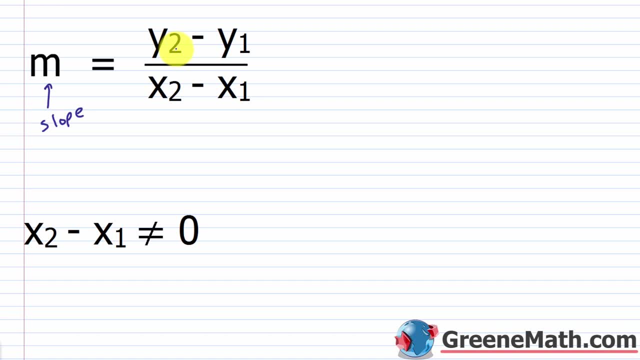 So let me explain real quick. We have Y and then we have a little 2, and then Y and then a little 1.. So it's a subscript in each case. So we say Y sub 2 minus Y sub 1.. This is just a way to notate. 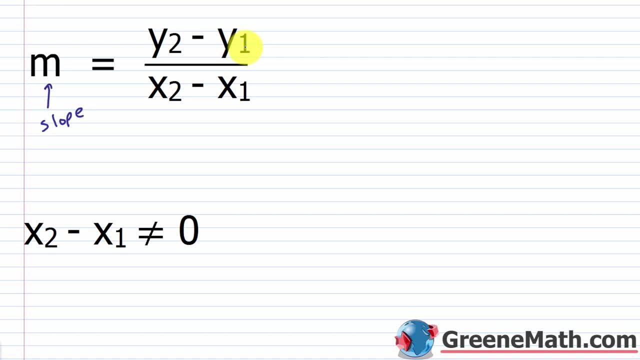 the different Ys that we have. We have two ordered pairs that we're working with, So X comma Y and then X comma Y. So I need to know which X I'm referring to and which Y I'm referring to. 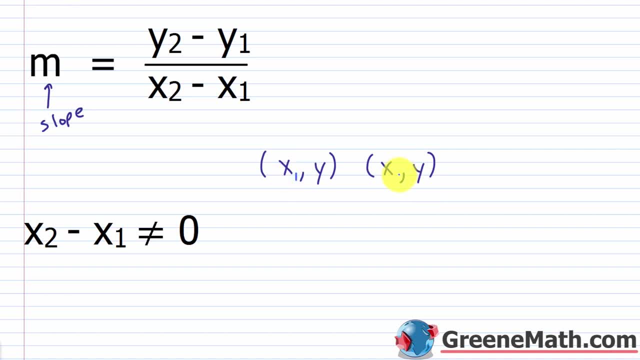 So the way we notate is we say, OK, this is X sub 1, and this is X sub 2.. This is Y sub 1.. This is Y sub 2.. And you don't mix and match, You don't say this is X sub 1,, Y sub 2, and this is X sub. 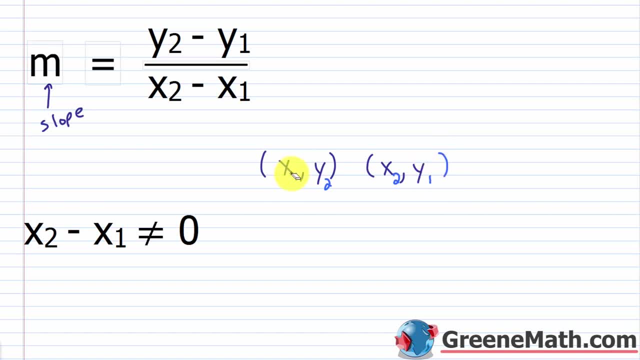 2, Y sub 1,, for example. You want to keep those notations consistent. So if this is X sub 1,, this is Y sub 1.. If this is X sub 2,, this is Y sub 2,. OK, That's going to help you with your formula. 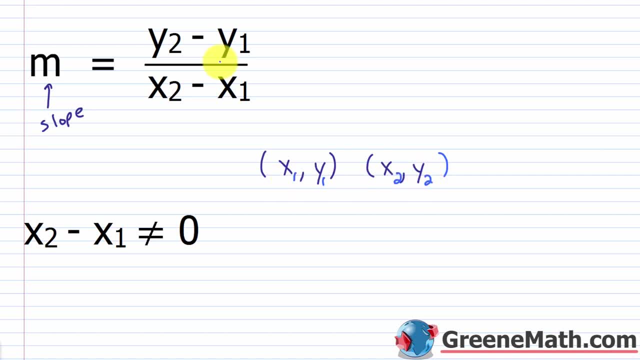 Now all I do, once I've notated things, is I just plug into the formula. OK, It's very, very simple. So Y sub 2 minus Y sub 1 is the change in Y values, or the rise. And then X sub 2 minus X sub 1 is the change in horizontal values or the run. So again, 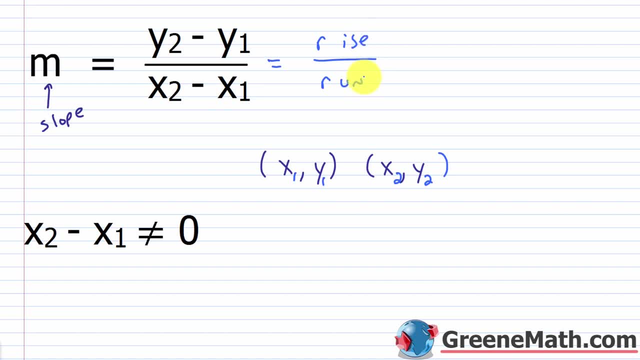 we see this rise over run. Now one little note before we kind of move on. we have that X sub 2 minus X sub 1 cannot be zero, And that's because if this is zero, here we'd be dividing by zero, and that's not allowed. All right, so let's go ahead and 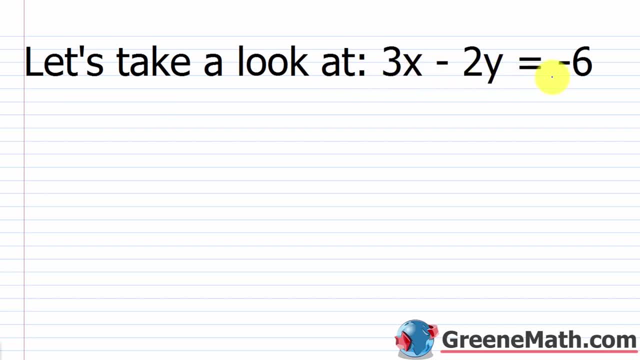 take a look at: 3X minus 2Y equals negative 6. So normally I would just give you two points and say: calculate the slope. but let's make it a little bit more interesting. So we have 3X minus 2Y. 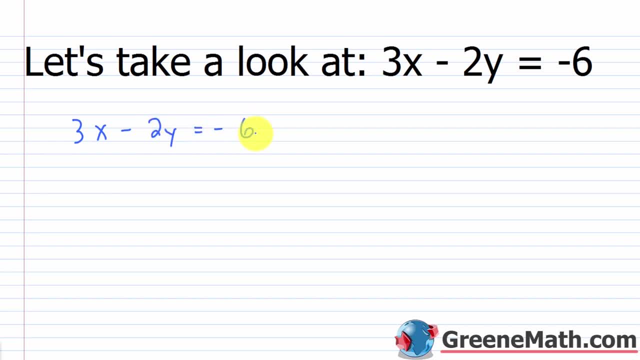 equals negative 6.. Just generate any two points that you want and plug them into the formula I just gave you. Now let's go ahead and use the X intercept and the Y intercept, because those are pretty easy to get. So for the X intercept, I plug in a zero for Y. So for my table of values, if I plug in a zero for Y, 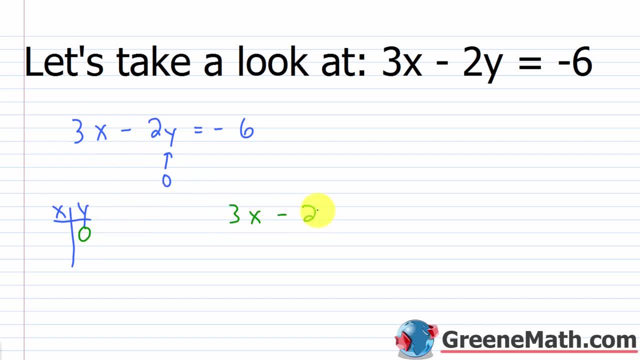 what would I get for X? I'd have 3X minus two times 0, equals negative 6, this would cancel to be zero and basically I'd have 3X equals negative 6.. Divide both sides by three and we get X equals. 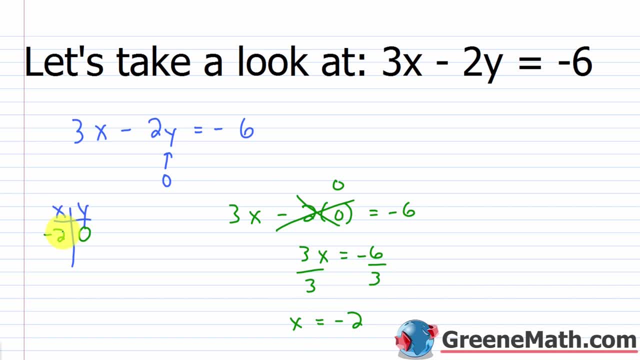 negative 2.. So X is negative 2, when Y is minus 2. y is 0.. Now for the y-intercept. I know that I want to plug in a 0 for x. So if I plug in a 0 here I would have 3 times 0 minus 2y equals negative 6.. So that would cancel. 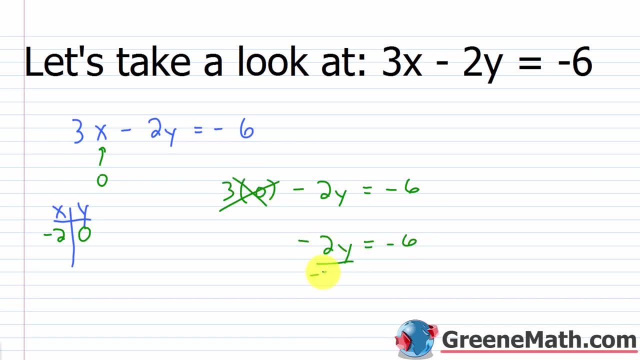 I'd have negative 2y equals negative 6.. Divide both sides by negative 2, and I'll have y equals 3.. So x is going to be equal to 0 when y is 3.. So now I have two points And 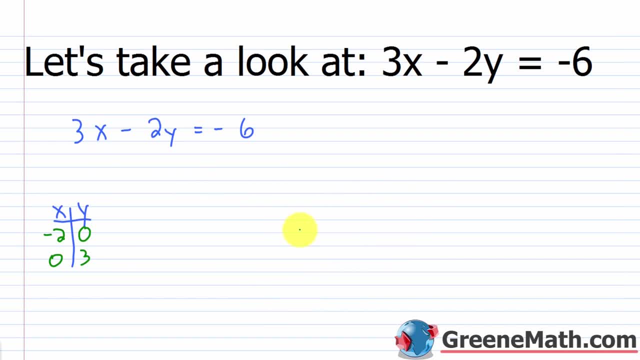 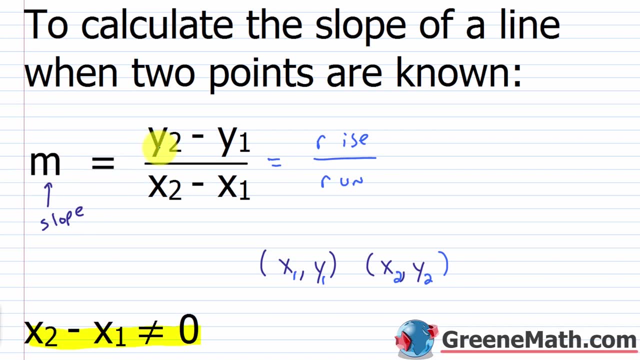 if I have two points, I have enough to calculate the slope. So I know you probably don't remember the slope formula from the other page, So let me scroll back And I want you just to copy it down. We have: m is equal to y sub 2 minus. y sub 1 over x sub 2 minus. 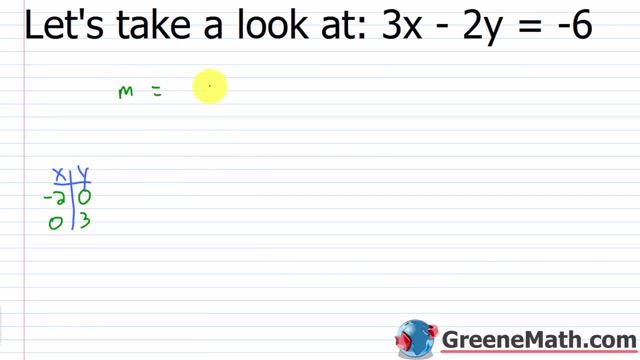 x sub 1.. So again that slope formula is: m is equal to y sub 2 minus y sub 1 over x sub 2 minus x sub 1.. Now I have two points here. I have negative 2 comma 0, and I have 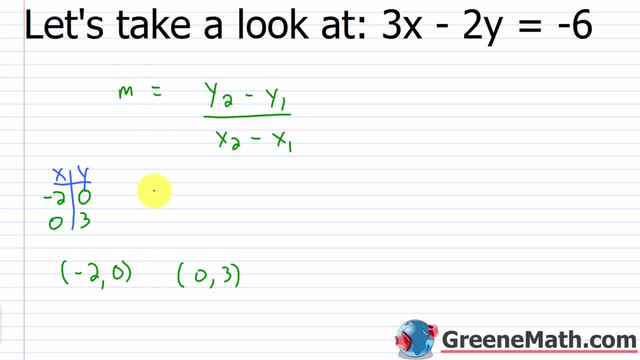 0, comma 3.. So the first question everybody asks- and you know I talked about this a lot when I taught Algebra 1, what point do I label as x sub 1, y sub 1? What point do I label? 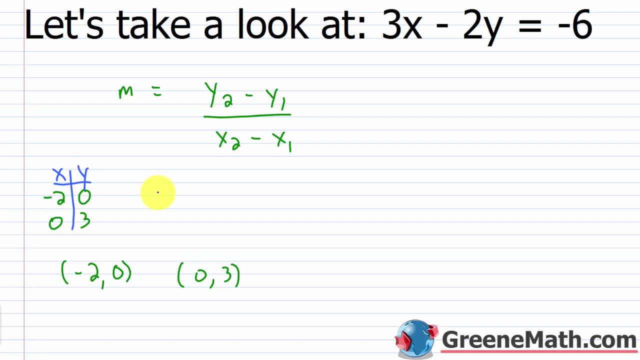 as x sub 2, y sub 2?. This is going to come up in your head And the answer to that is: it doesn't matter. Write that down now, because you're going to ask that question again if you haven't asked that question before. 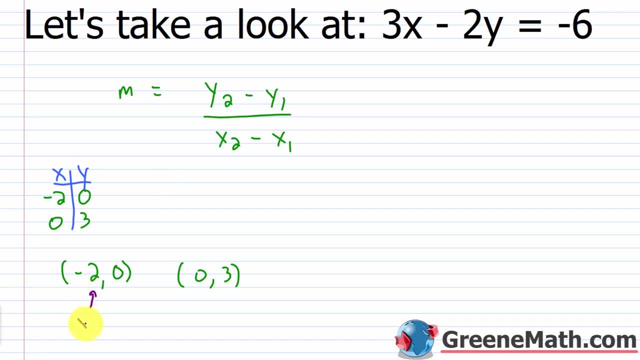 If I start out and say this is x sub 1, and this is y sub 1, and this is x sub 2, and this is y sub 2,, I would get the same answer as if I changed this and I said this is x. 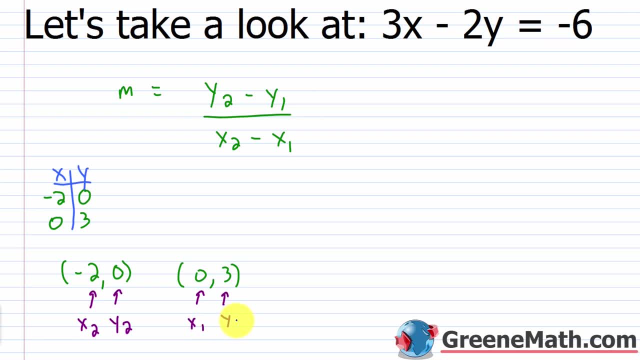 sub 2, this is y sub 2, this is x sub 1, this is y sub 1.. What I want to do is just make sure I'm consistent with my notation. So, in other words, if this is x sub 2, this is. 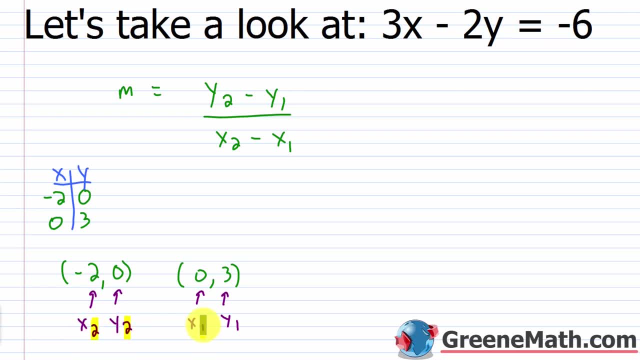 y sub 2.. I have a 2 in each case. If this is x sub 1, this is y sub 1.. I have a 1 in each case. So now that we've got that covered, we just plug into the slope. formula y sub 2 is 0,. 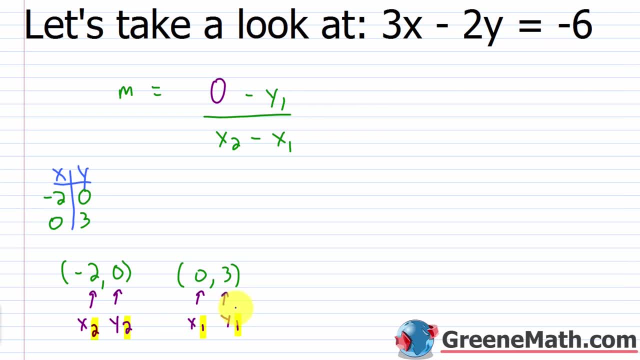 so I'm just going to erase this and put a 0.. y sub 1 is 3,. erase this and put a 3.. x sub 2 is negative 2,, so erase this and put negative 2.. And then x sub 1 is 0,, so erase. 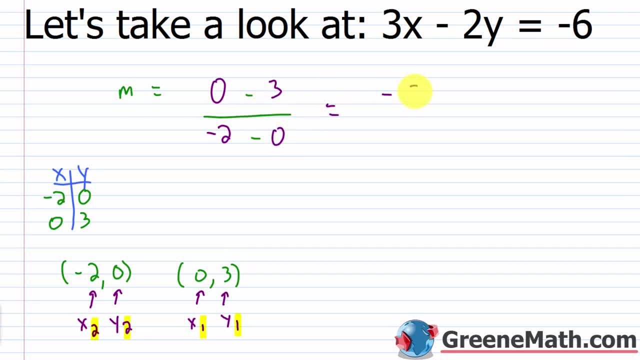 this and put a 0. So 0 minus 3 is negative 3. Negative 2 minus 0 is negative 2. Negative 3 over negative 2 is 3 halves. So what does this mean? m equals. 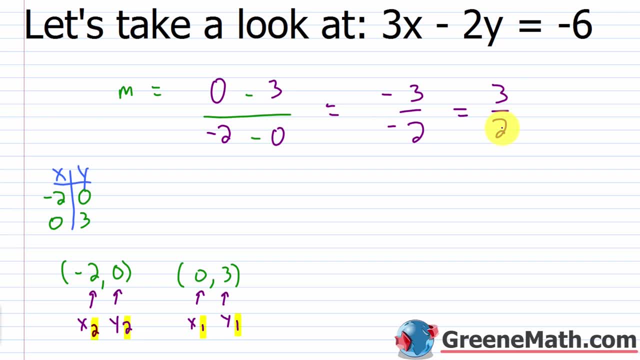 3 halves. Well, a slope of 3 halves means that again I go back to the definition. I rise 3 units for every 2 units that I run. So graphically, if I started out at a point on the line and I went up 3 units and I go to the right 2 units, I'm going to go back. 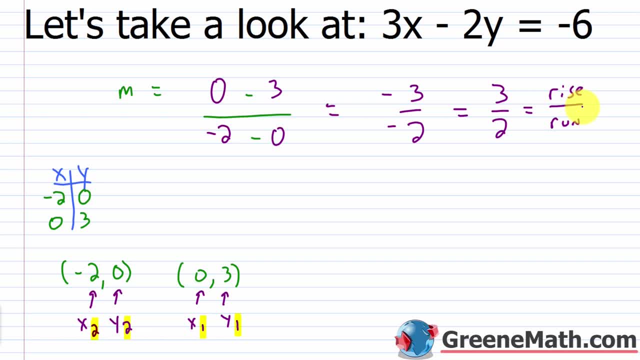 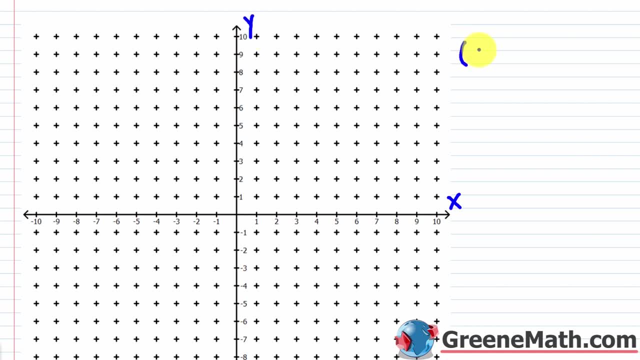 to that line. So let me graph this line and we're going to show you that. So again, this is my x axis, this is my y axis, and I had 2 points, I had 0 comma 3, and I also had negative 2. 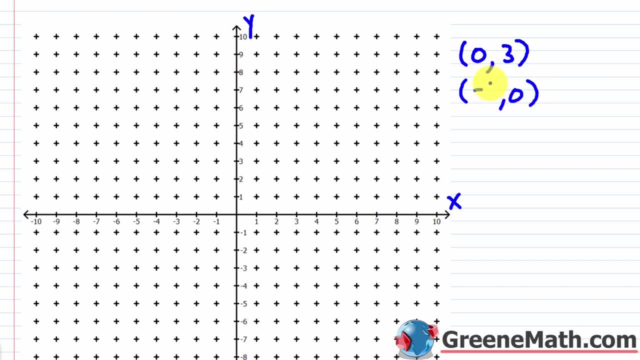 comma 0. And I know that when we were graphing I said to do 3 points and you can do that if you want. but I already know that this is correct, so I'm not going to waste your time by getting a third point. So 0 comma 3 is right here. Negative 2 comma. 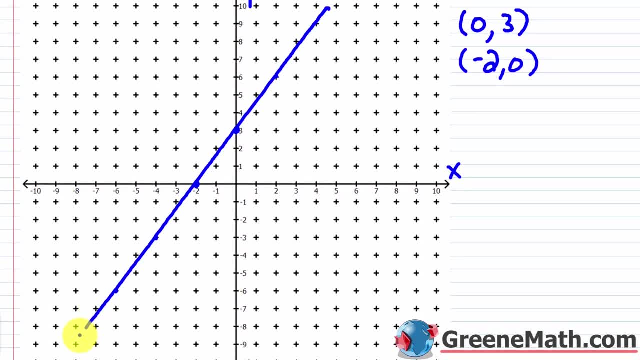 0 is right here. Okay, again, this is the graph, for 3x minus 2y is equal to negative 6.. Now we talked about the fact that this had a slope. m is equal to 3 halves, So I can start out at. 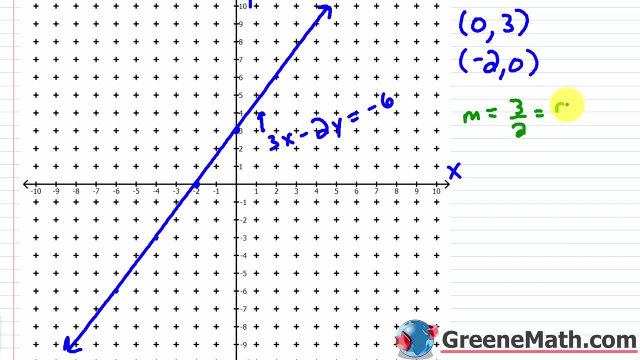 any point on this line. Remember, this is the rise over the run. Okay, so now I'm going to show you this. If I start out at this point, if I rise, 3 units, so 1,, 2,, 3, and 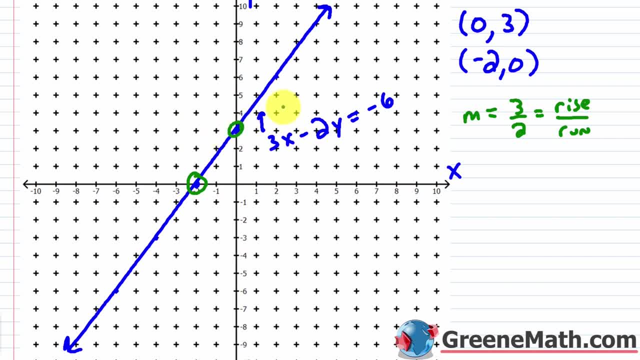 I run 2,, 1,, 2,. I'm back to the line. Rise 3, 1,, 2,, 3, run 2,, 1,, 2, back to the line. Rise 3, 1,, 2,, 3, run 2, back to the line. It also works a different way, If I think. 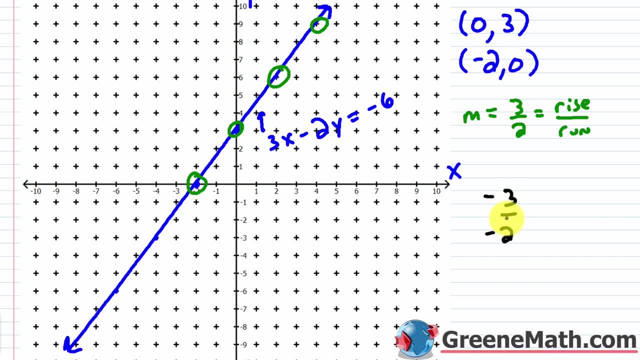 about 3 halves as negative. 3 over negative. 2, negative over negative is positive, so it's the same thing. Similarly, I start at a point and I go down 3, so 1,, 2,, 3, that's my rise and I run negative. 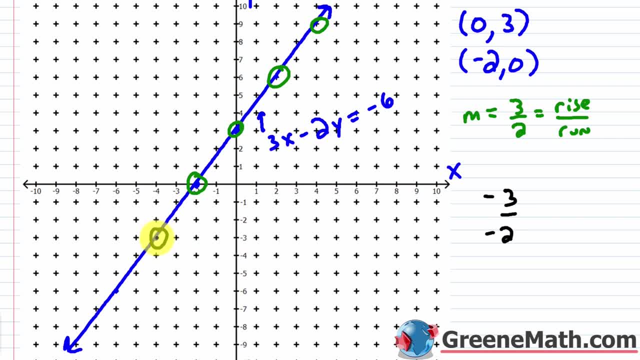 2.. So I go to the left: 2, 1, 2,. back to the line Fall: 3, 1,, 2,, 3, go to the left: 2, right here, That's what slope is telling us. For every 3 units, I rise, I run 2.. 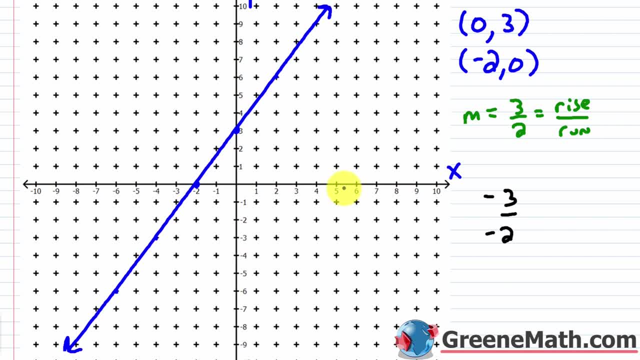 All right. so let me show you one other thing. I want to show you how this procedure where we have m equals again y sub 2 minus y sub 1.. All right, so let me show you how this procedure where we have m equals again y sub 2 minus. 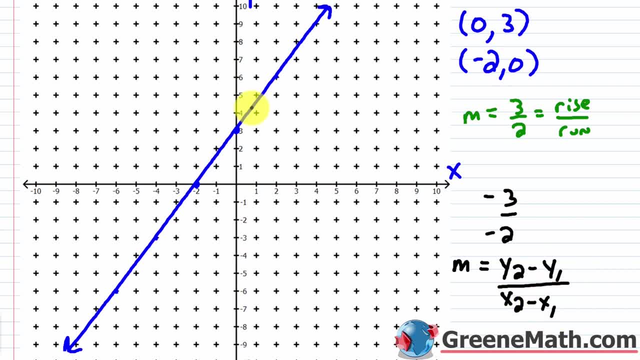 y sub 1, works on the coordinate plane. So again, if we use the point 0, 3, and we use the point negative 2, 0,, when I think about y sub 2 minus y sub 1,, the y value, let's: 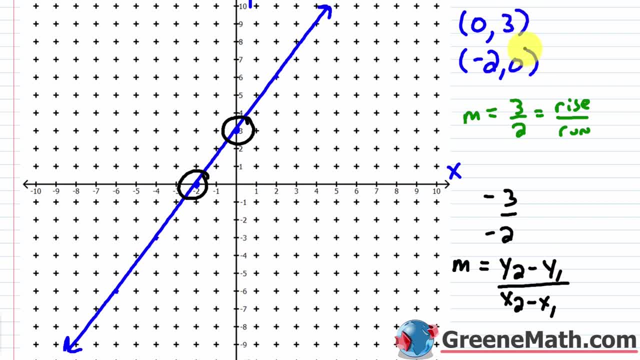 just say from here is 3, and let's say from here it's 0.. So 3 minus 0, that gives me the rise or the change in y values from here to here. All right, that's my change in y. 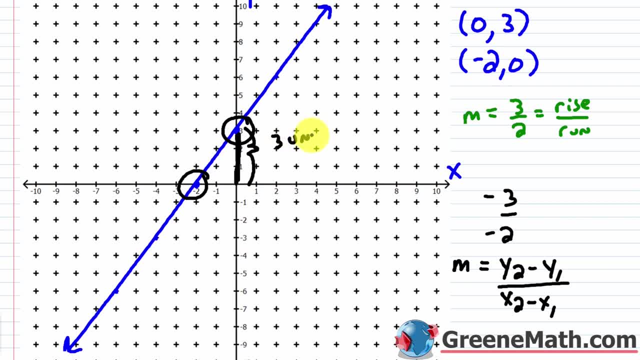 This distance here, So that's 3 units. Now my change in x values. think about 0 minus a negative 2, which is basically 0 plus 2, or 2.. I'm going from here to here, So I'm. 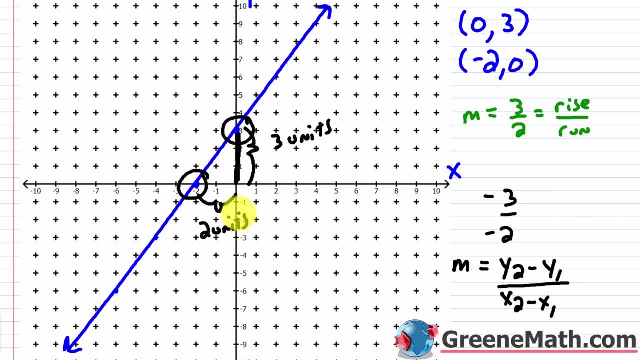 traveling 2 units And it's easy to see that the slope again it's. I go 2 units to the right and 3 units up, So I rise 3, run to the right 2, or 3 units up, So I rise 3,. 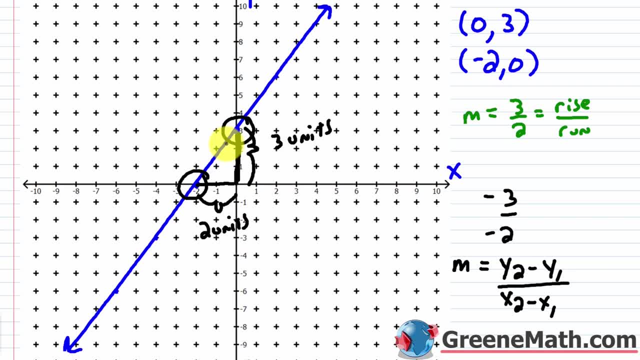 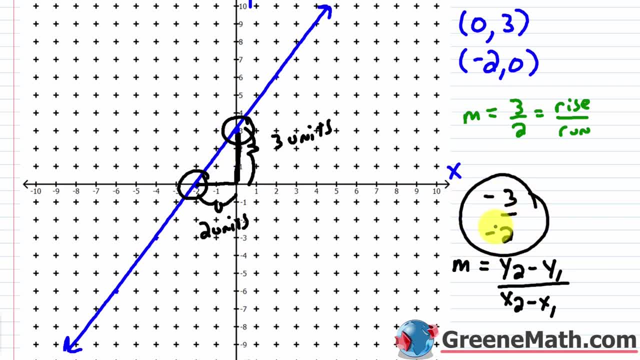 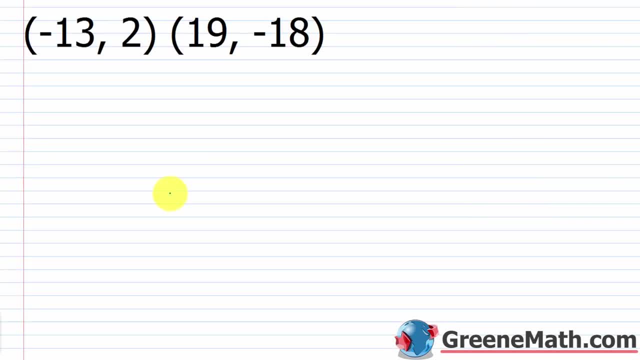 up All right. So now that we understand kind of the concept behind this, let's just crank out a few examples. So let's say you get your homework or your test and you're given these two points and they say: calculate the slope. 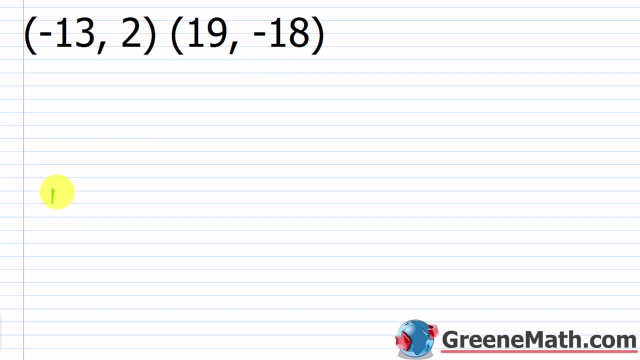 Well, again you're going to use the slope formula. So m is equal to y sub 2 minus y sub 1 over x sub 2 minus x sub 1.. So I just generically label: one point is x sub 1, y sub 1.. 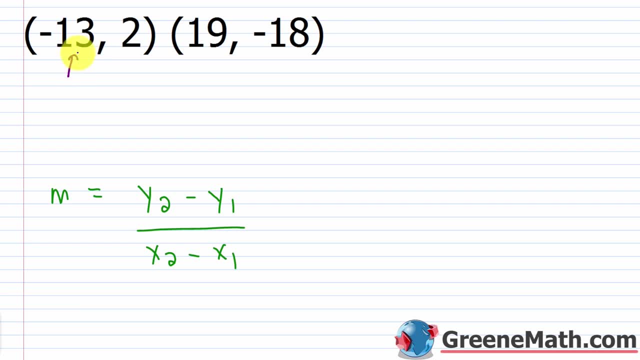 The other is x sub 2, y sub 2.. Doesn't matter which is which. So this is x sub 1, y sub 1.. This is x sub 2, y sub 2.. Again, I could have switched that up. 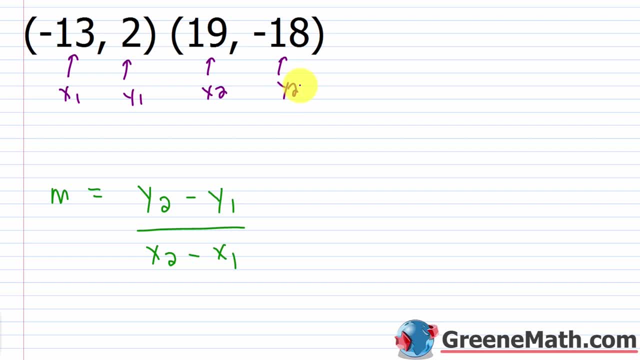 It would make no difference in the calculation. So for y sub 2, I have negative 18.. For y sub 1, I have 2.. For x sub 2, I have 19.. For x sub 1, I have negative 13.. 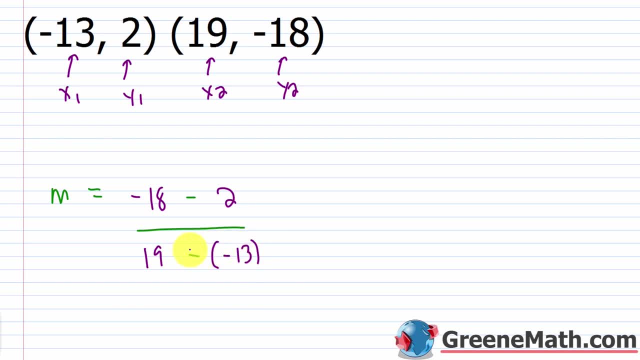 Be very careful with plugging in negatives here, because you have that minus, So you want minus and negative 13.. All right, so this is equal to negative. 18 minus 2 is negative 20.. This is over 19 minus a negative. 13 is the same thing as 19 plus 13.. 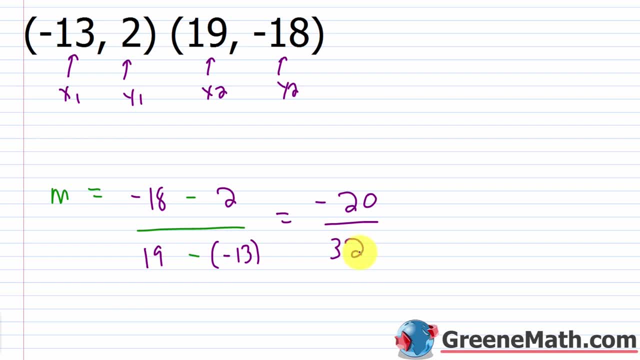 19 plus 13 is 32.. So you get negative 20 over 32.. Of course, we can reduce this. Each is going to be divisible by 4.. Divide this by 4, you get 5.. Divide this by 4, you get 8.. 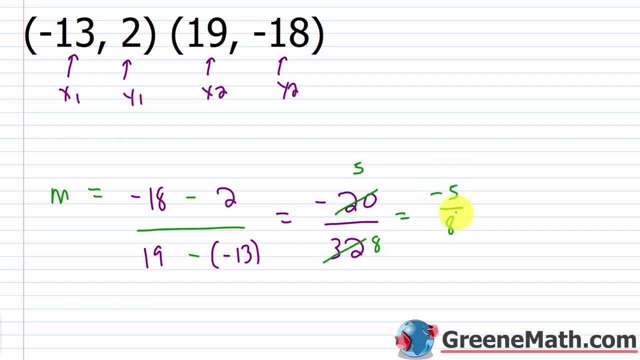 So this equals negative 5 eighths. So what this means is that my slope, or m, is negative 5 eighths. So I would rise By negative 5 for every 8 units that I run. And when we think about negatives here, there's a couple different things we can think about. 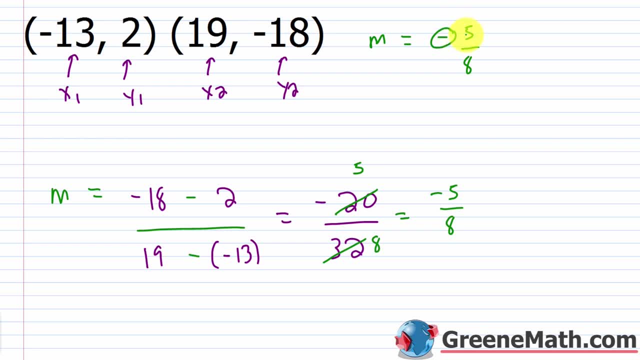 First off, remember a fraction. if the numerator is negative and the denominator is positive, I can switch that up. So when I think about slope, I can say that the rise is negative 5 and the run is 8.. Or I could say: the rise is positive 5 and the run is negative 8.. 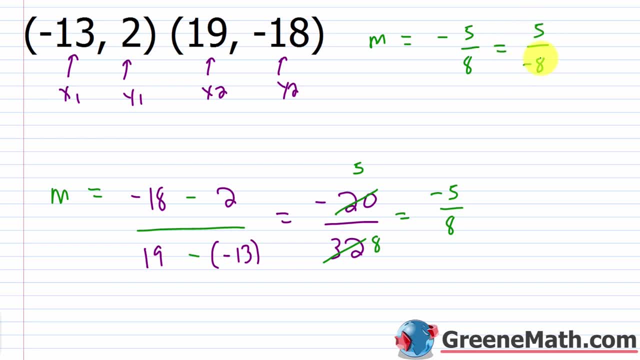 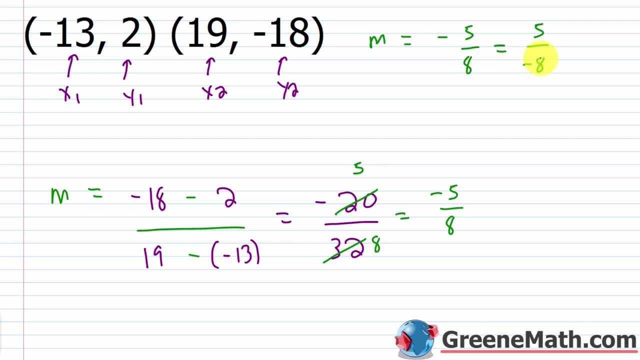 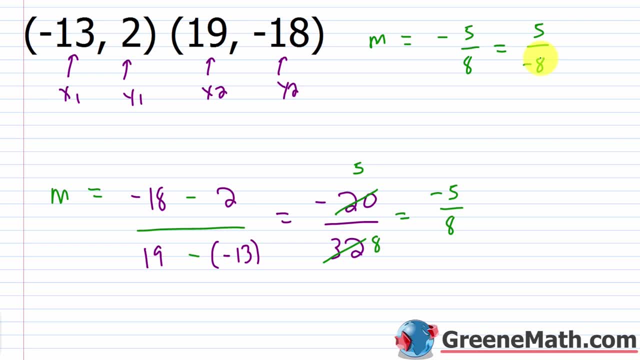 Okay, If you're on a vertical number line, I increase by going up right, Going north. I decrease by going down or going south. If I am on a horizontal number line, a typical number line, as I go to the right, I'm increasing. 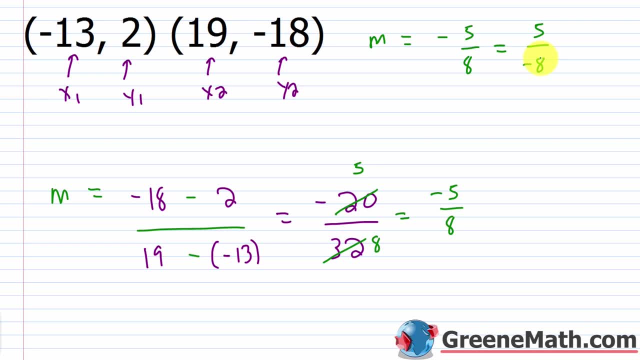 As I go to the left I'm decreasing. Okay, So just relate that All right. So let's take a look at another example. Let's say you have 15 comma negative 10 and 10 comma 6.. So again, let's label these points here. 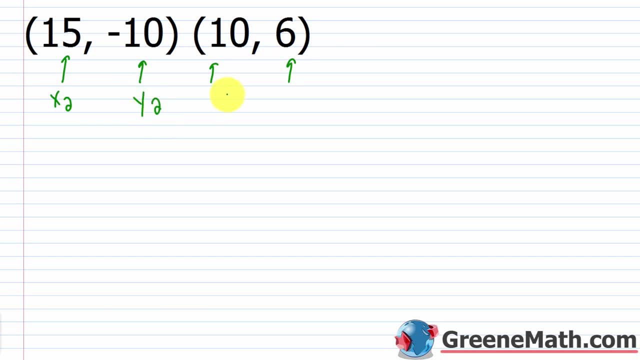 And I'm going to switch it up and say: this is X sub 10.. This is Y sub 2.. This is X sub 1, Y sub 1.. And I just plug into the formula: So M, the slope is equal to Y sub 2,, which is negative 10, minus Y sub 1,, which is 6,. 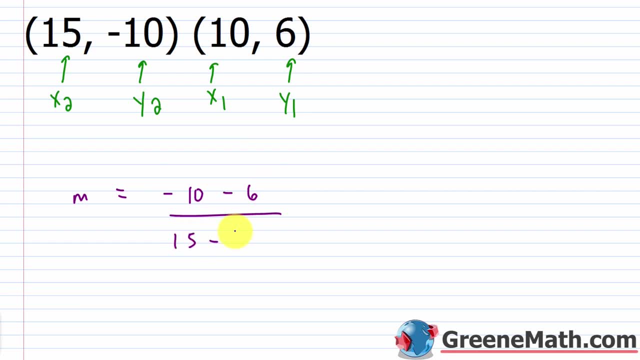 over X sub 2,, which is 15,, minus X sub 1,, which is 10.. Again, I'll write the formula here: It's Y sub 2 minus Y sub 1, over X sub 2 minus X sub 1.. 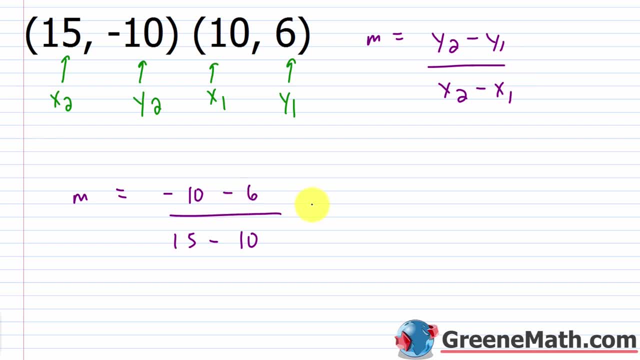 Again, rise over run. So negative 10 minus Y sub 1. It's going to be negative 16 over 15 minus 10, which is going to give me 5.. So I can't reduce that any further. My slope is just negative 16. fifths. 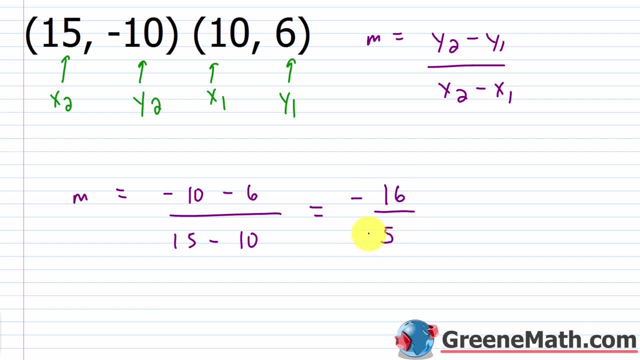 So again, this tells me that I fall 16 units for every 5 that I go to the right. Or I could switch this up and say that I increase 16 units for every 5 that I go to the left. I can have 16 over negative 5 as well. 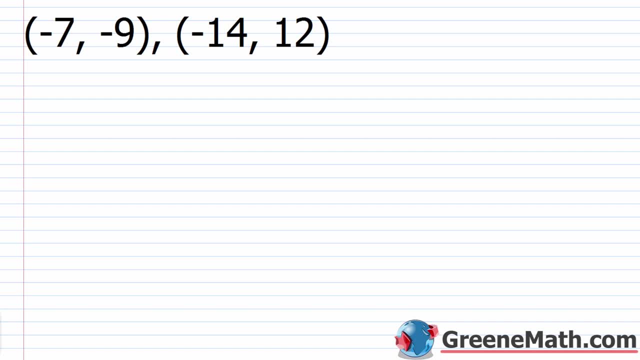 All right, Let's take a look at another example. So we have the ordered point, All right, So we have a slope formula. So we take a look at the slope formula. This is the slope formula that we're using. We're going to use the slope formula and the order pair: negative 7 comma, negative 9. 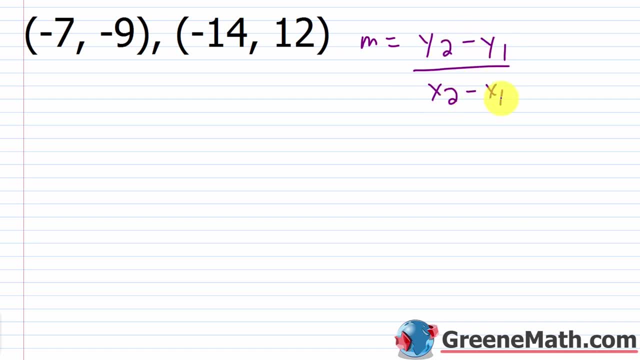 and the order pair: negative 14 comma 12.. So again, I'm just going to use my slope formula. So M is equal to Y sub 2 minus Y sub 1 over X sub 2 minus X sub 1.. Again, copy that down and refer to it as we're working the problems. 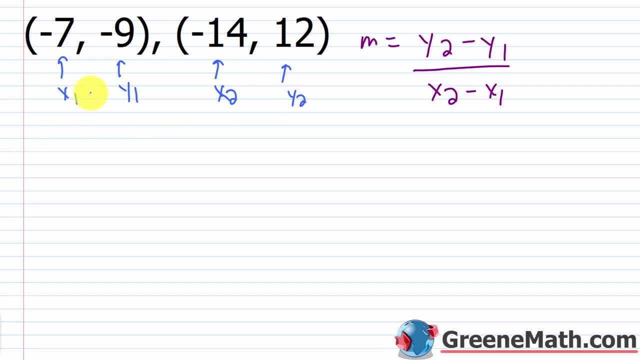 So I label. The only thing that matters is if I put this as a 1,, this is a 1.. This is a 2,, this is a 2.. Don't mix that part up. but you can label either one as x sub 1,, y sub 1, and the other. 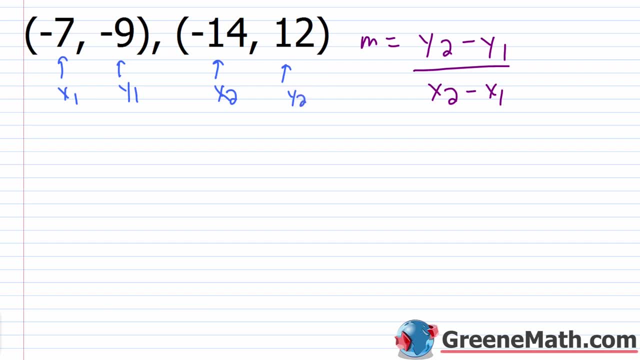 as x sub 2, y sub 2.. Doesn't matter, All right. So m is equal to. for y sub 2, I have 12, then minus for y sub 1, I have negative 9, so it's minus a negative 9,. okay, be careful there. then over for x sub 2: I have negative. 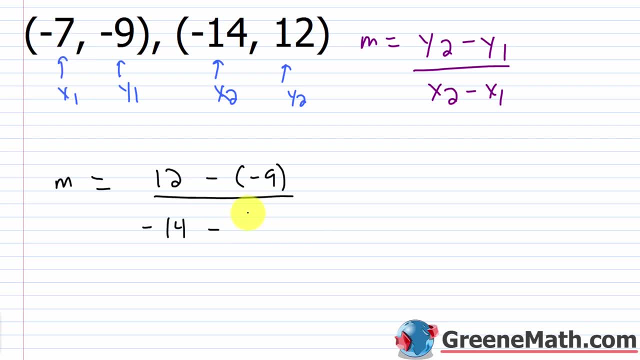 14, and then minus for x sub 1, I have negative 7, so minus a negative 7.. So 12 minus a negative 9 is the same as 12 plus 9, that's 21.. Negative 14 minus a negative 7, that's basically negative 14 plus 7, so that's negative 7.. 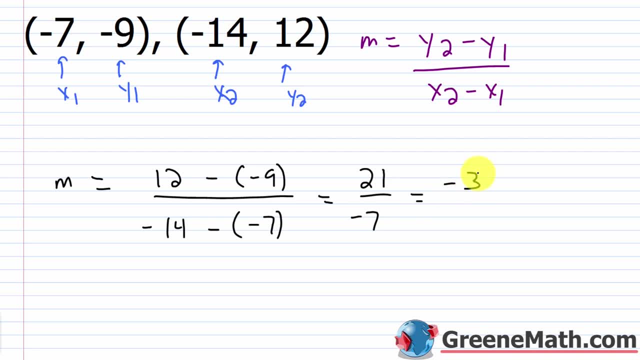 So 21 over negative 7 is negative 3.. Now typically with slope we'll say negative 3 over 1, so we can still refer to rise over run. My rise is negative 3.. My run is 1.. So if I'm on a graph and I'm at a point there, I can fall 3 units and run to the right 1,. 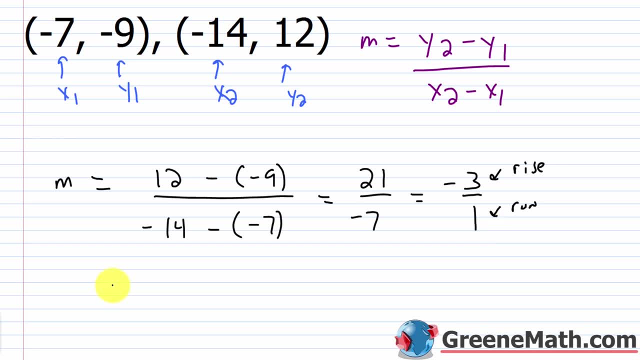 and I'm back to the line. Or again, another thing I can do: I can switch this negative, I can say this is 3 over negative 1, so I can say the rise is 3 and the run is negative 1.. 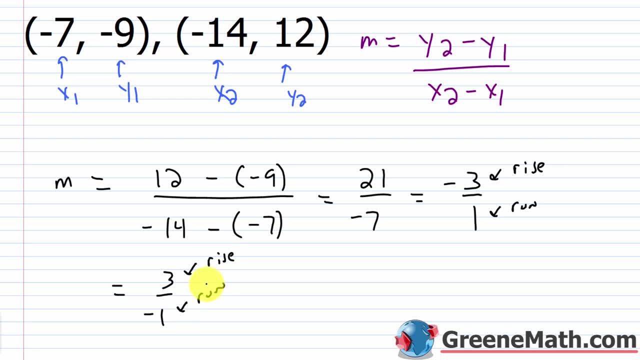 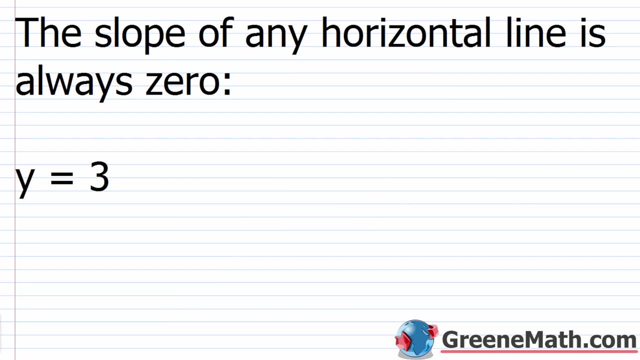 So now if I'm at a point on the line, I can go up 3 and to the left 1.. Okay, So pretty easy overall to find the slope of a line if you're given two points. If you're not given two points, if you're just given the equation, then you can just. 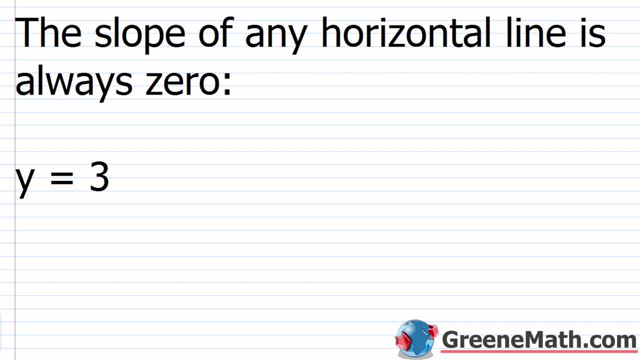 calculate two points, then plug it into that slope formula. Super, super easy to do, All right. so now let's talk about a few special case scenarios. So the slope of any horizontal line is always 0. So why is that the case? 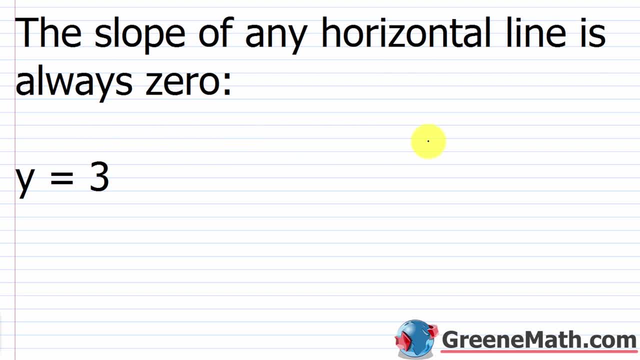 Well, we know a horizontal line just goes straight across, So its steepness would be nothing right. It's not rising at all as it's moving to the right, So it would basically be 0 over whatever, 0 over 1, or 0 over 25.. 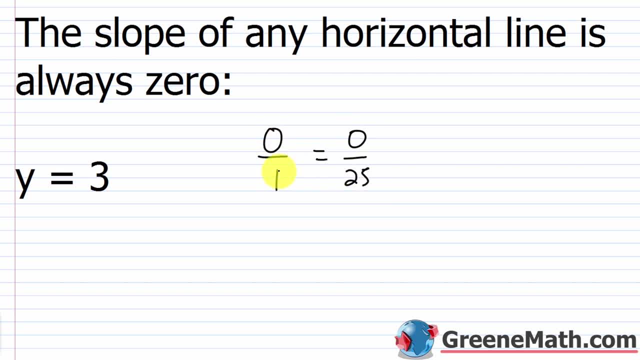 So I go 0 units up for every 1 unit, I go to the right, or I go 0 units up for every 25 units, I go to the right, And this doesn't look correct. 0 over 1 equals 0 over 25, yeah, 0 divided by any non-zero. 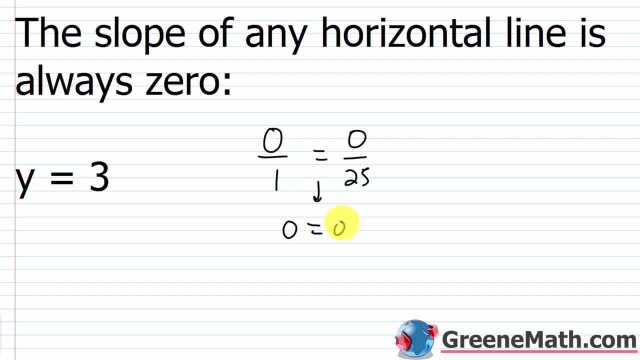 number is 0. This is 0 equals 0, right Have a steepness or slope of 0. So you can use the slope formula to calculate this. Remember I can generate two points by choosing a value for x arbitrarily. 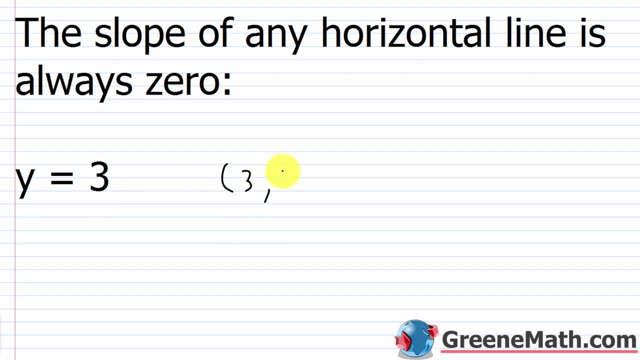 Let's say it's 3,, for example. So x is 3, y is 3.. X is, let's say, 10.. Y is 3.. No matter what I choose for x, y will always be 3.. 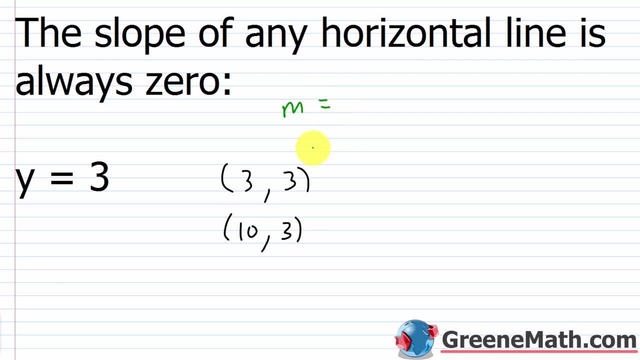 So then if I plug that into my slope formula, So if I plug that into my slope formula, m is equal to: and let's say this is x sub 1, y sub 1, and this is x sub 2, y sub 2.. 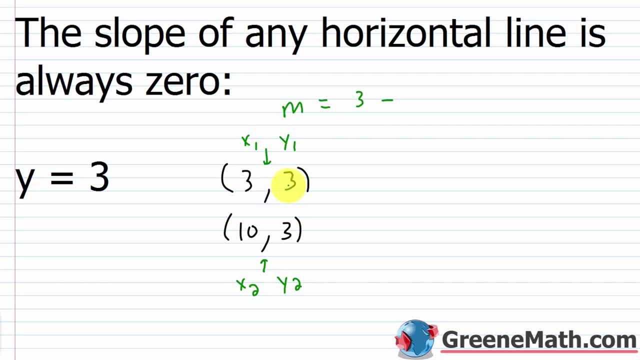 So m is equal to y sub 2,, which is 3, minus y sub 1,, which is also 3, that's where you get your 0 from over x sub 2,, which is 10, minus x sub 1,, which is 3.. 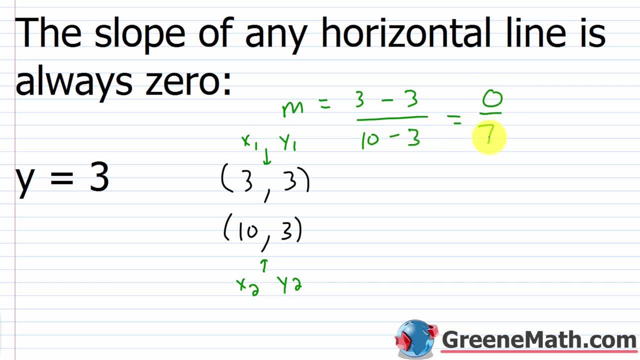 So 3 minus 3 is 0, over 10 minus 3, which is 7.. 0 over 7 is obviously 0.. 0 over 7 is obviously 0.. 0 over 7 is obviously 0.. 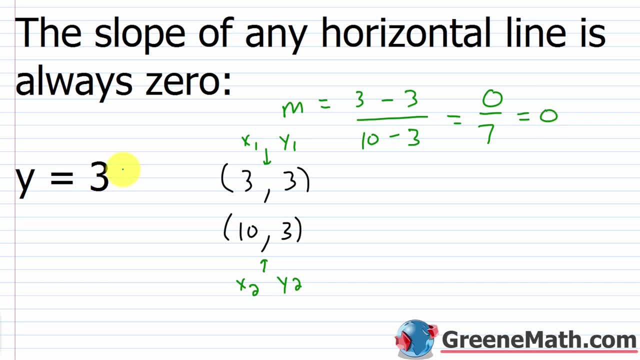 0 over 8 is definitely 0.. The point you have said is 0, and yourvariance as you disassociate yourself from your artwork shape of your rise, will always be 0, because the value Y for the 2 points you choose is. 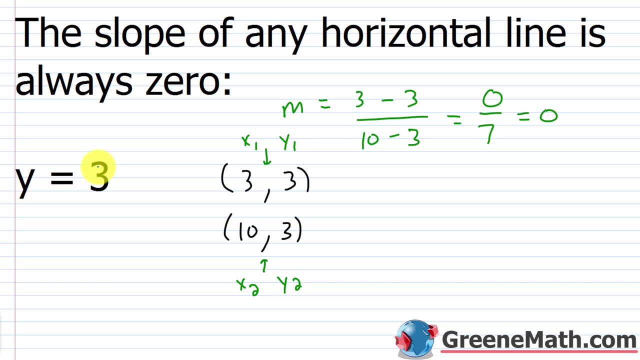 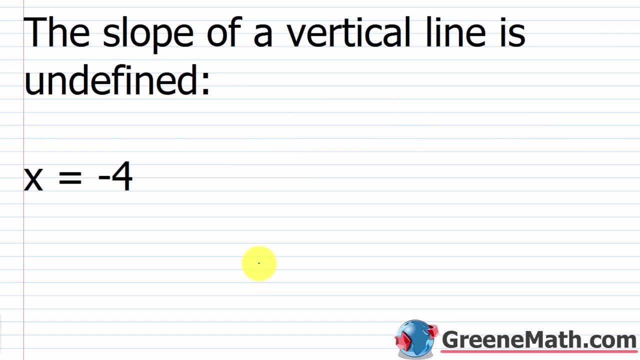 always the same. The same sum is always going to give you 0.. 5 minus 5 is 0.. 20 minus 20 is 0.. 2 million minus 2 million is 0.. You know so on and so forth. 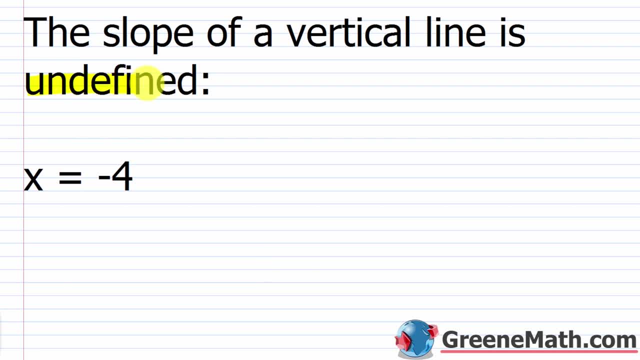 You know so on and so forth. So the other special scenario would be the slope of a vertical line. So the slope of a vertical line is undefined. So why do you think that is our slope formula We have? m is equal to y sub 2 minus y sub 1 over x sub 2 minus x sub 1.. If x. 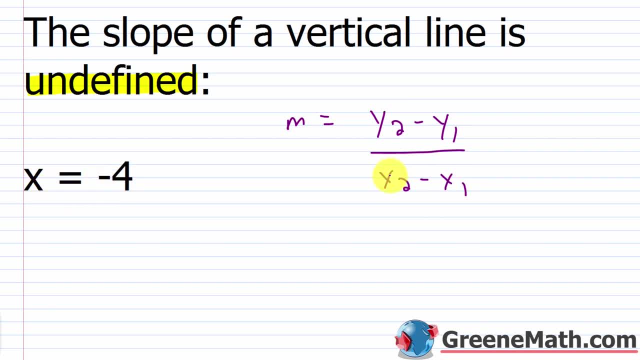 always equals negative 4,. for x sub 2, it's going to be negative 4.. For x sub 1, it's going to be negative 4.. Negative 4 minus a negative 4 is negative 4 plus 4.. That's 0.. So I'm going to 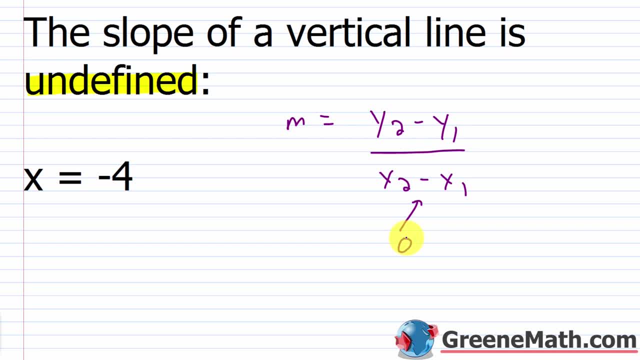 have division by 0, which is not allowed. It's undefined. So that's why we say the slope of a vertical line is undefined. And again, if you want an example of that, let's say you're given a problem where you have something like negative 4 comma 3, and let's say you have negative 4 comma. 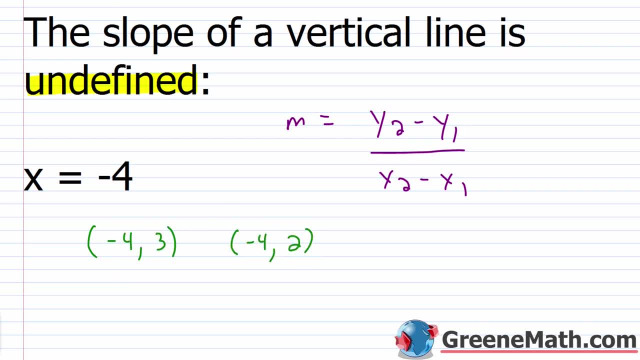 2.. If you see the same value for each x, you know you have an undefined slope. Let's say this is x sub 1, y sub 1, and this is x sub 2, y sub 2. Just try plugging it in, So for y sub 2, you get 2.. 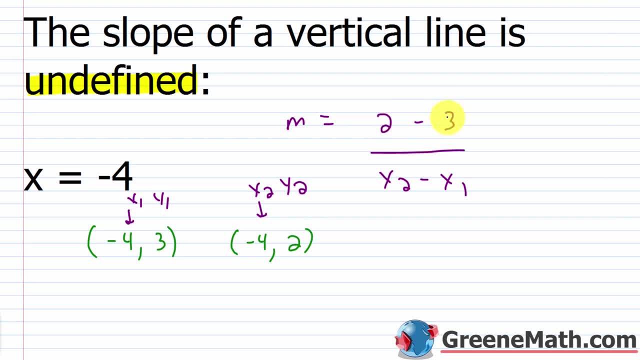 For y sub 1,, you get 3.. For x sub 2,, you get negative 4.. And for x sub 1,, you also get negative 4.. And remember, minus a negative is plus a positive. So really this is negative 4 plus 4.. 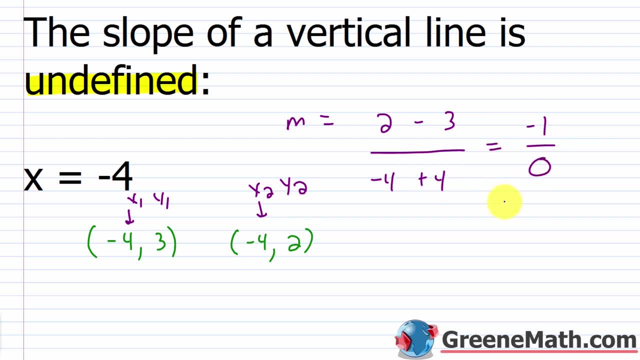 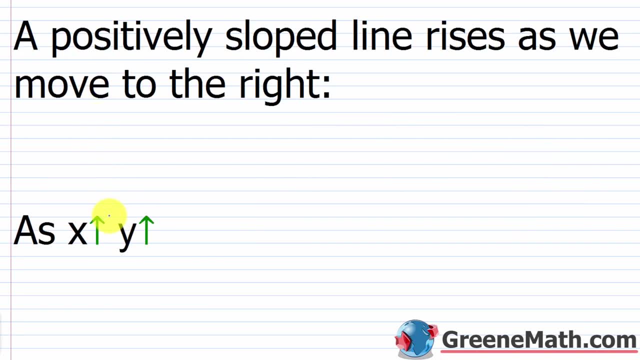 So 2 minus 3 is negative 1, but it's over 0. So again, this is undefined. All right, so a couple of just key points. on slope: So a positively sloped line rises as we move to the right. So if you see a slope, that's something like three-fifths. 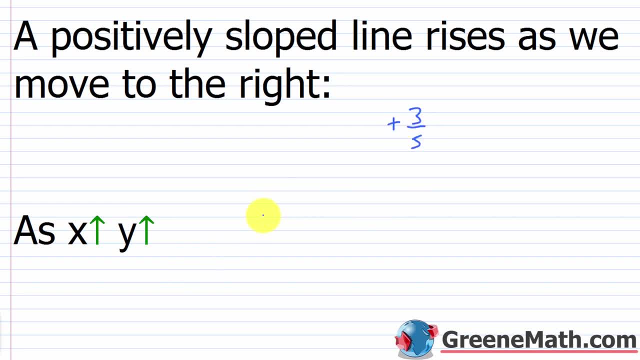 I know this is positive. I know that as x increases, so as we move to the right, that line's going up. So a positively sloped line looks something like this: Again, as we're moving to the right, as x is increasing, the values for y are increasing. 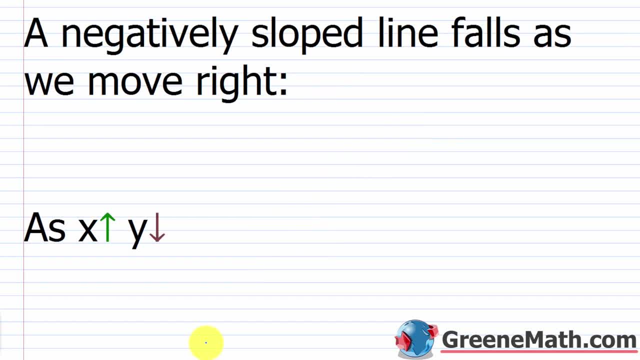 So I'm going up. Then, similarly, a negatively sloped line falls as we move to the right, So as x increases, in this case, a negatively sloped line would have a y that decreases. So you'd see something With a negative slope. you have a negative. Let's say it was negative. 3 or let's say negative. 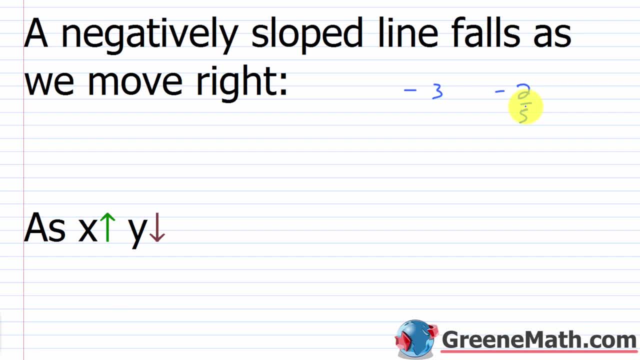 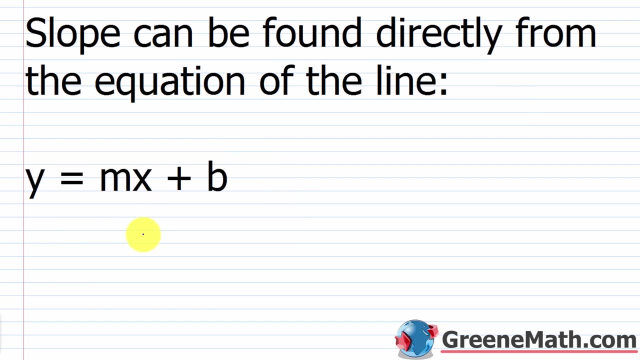 two-fifths or something like that. That type of line again falls as it moves to the right. So it looks something like this: As we move to the right, as x increases, the y values are decreasing. All right, so now let's get into something that is going to probably piss you off. 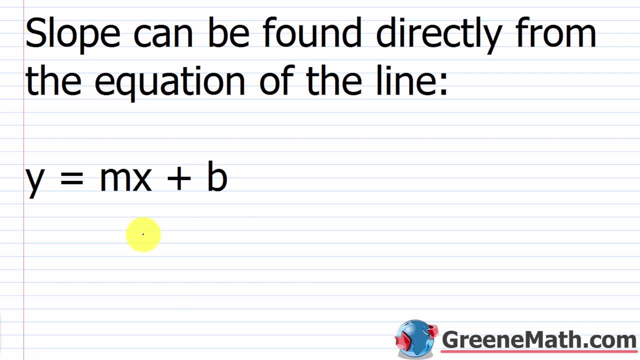 Slope can be found without using the slope formula. It can be found directly from the equation of the line. So I know a lot of students. they get these equations, they go through, they figure out these points and they plug in the slope formula. They do all this work and then they figure out. 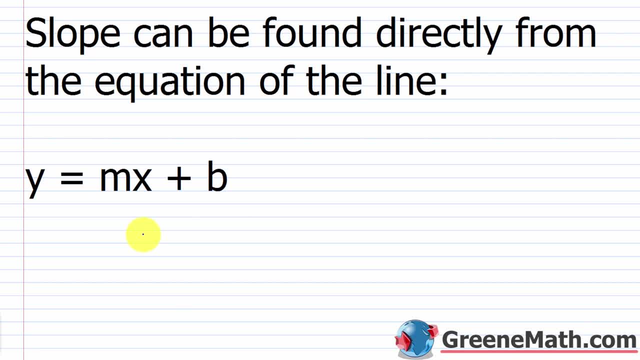 that it's so easy to just solve for y. Often they get really, really mad, So hopefully you're not upset about that. It's important to understand all the techniques that we have in math, because sometimes you're not given the equation, Sometimes you have to generate it. I have here that y equals. 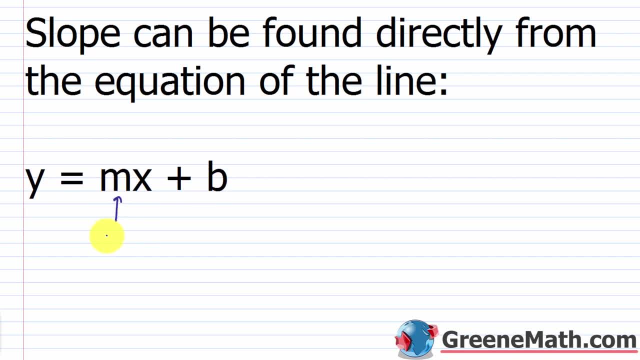 mx plus b. You remember that m stands for slope. To solve the equation for y, the coefficient of x is the slope, and I'll prove that to you in a second. b is something that's new for us, not if we took Algebra 1, but if we haven't seen this before. 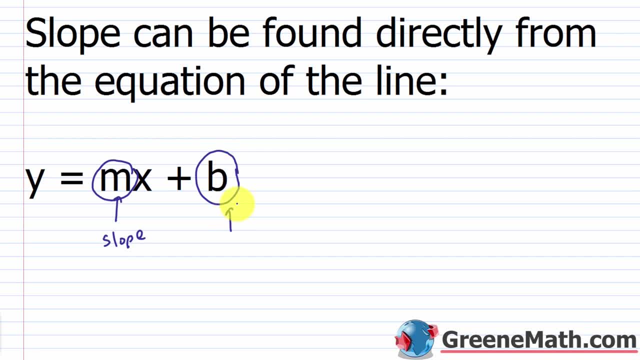 b is basically the y coordinate for the y-intercept. So in other words, if I plugged in a 0 for x, m times 0 would be 0, so this would disappear. I'd have y equals b. So the coordinate 0 comma b is your y-intercept. 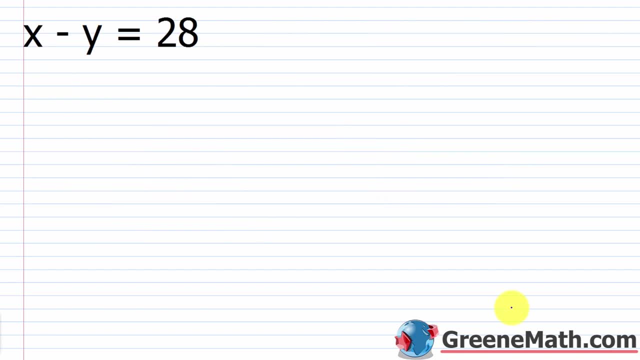 Alright. so let's say we're given an equation: x minus y equals 28. And I tell you to find the slope. So all I'm going to do is just solve it for y. So I want to isolate y on one side. So the first thing. 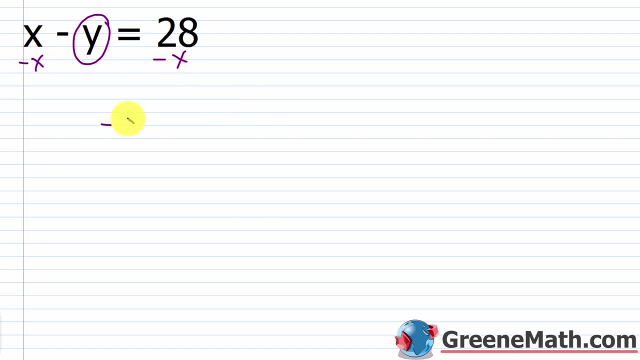 I'm going to do is subtract x away from each side, So I'll have negative y is equal to negative x plus 28.. Then I just want to get rid of the negative, So let's divide both sides by negative 1. And so this will cancel. with this, I'll have: y is equal to negative x plus 28.. 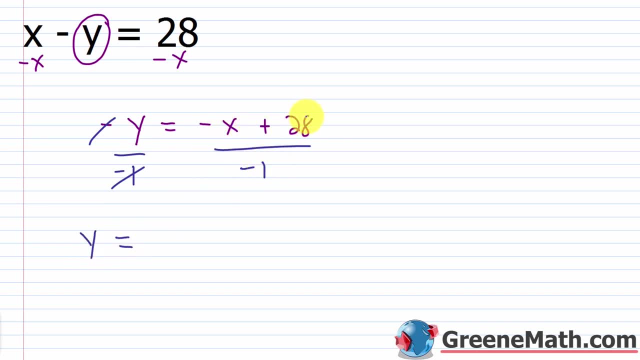 So let's divide both sides by negative 1, and so this will cancel. with this I'll have: y is equal to negative x plus 28.. You think about this as dividing each by negative 1.. So negative x is divided by negative 1, so that's x. 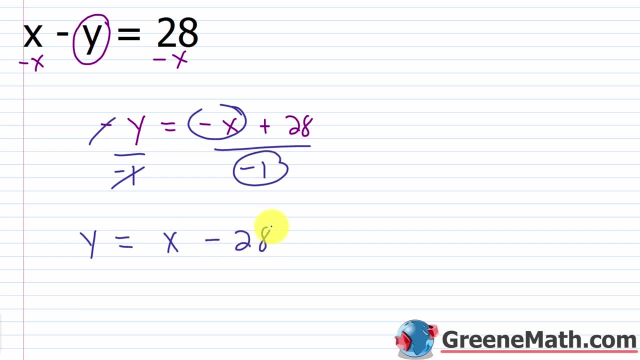 And then 28 is divided by negative 1, that's minus 28.. So y equals x minus 28.. So the coefficient of x here is understood to be 1.. So that's my slope, And my y-intercept would occur where: 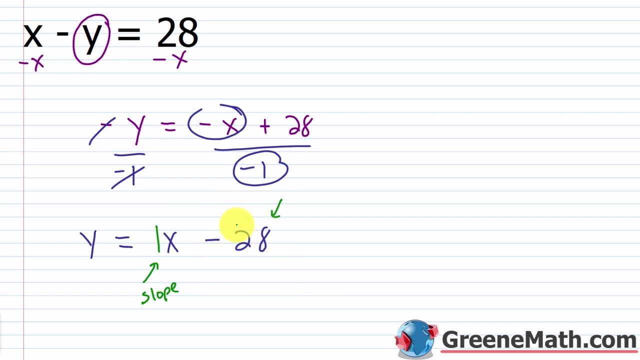 Well, if I plugged in a 0 for x, I'd have negative 28 as my result for y. So my y-intercept is at 0, negative 28.. Again, this is m. this is b. When you think about b, you want to think about the sign that's in front. 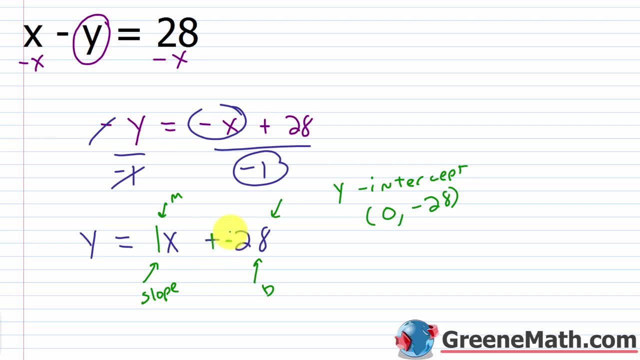 I could really write this as plus negative 28 if I wanted to, so that's why we write 0, negative 28.. All right, so let me prove to you that this works. I'm going to prove to you that the slope is 1 here. 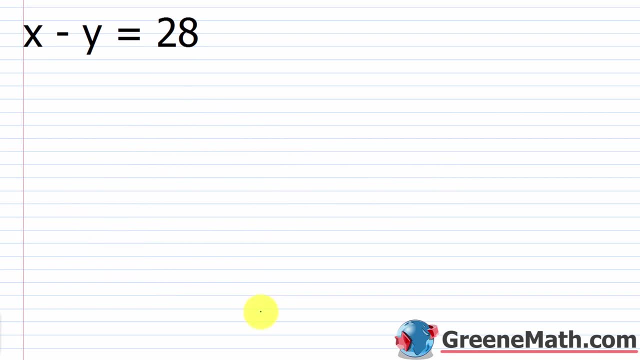 So let's say you didn't know, You didn't know what I just taught you And you're given this and your only technique is to use the slope formula. So you generate two points. Let's say that you generate I don't know. let's say x is 12.. 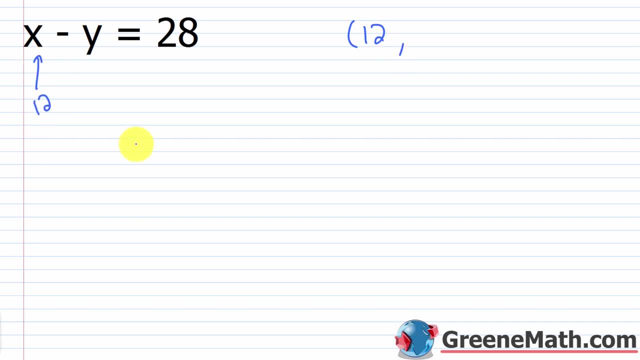 What would y be? I'll plug in a 12 there. So then I'd have 12 minus y equals 28.. I would subtract 12 away from each side of the equation That cancels. I have negative. y is equal to 28 minus 12 is 16.. 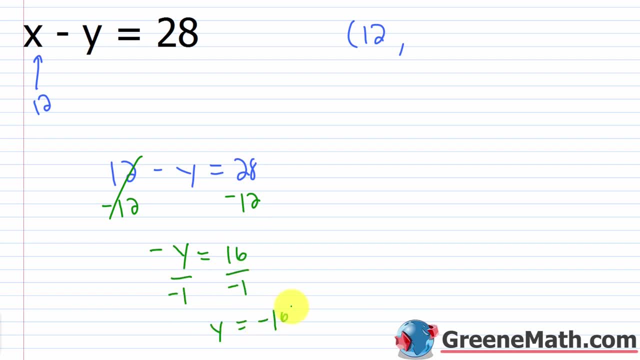 Divide both sides by negative 1. You get y is equal to negative 16.. So if x is 12,, you get y is equal to negative 16.. As another point, let's just say we pick- I don't know how- about 14?? 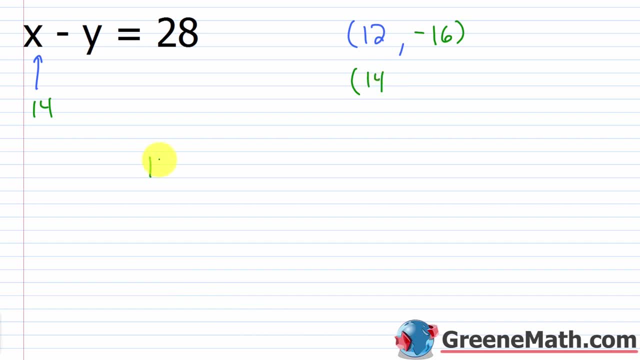 So if x is 14, what's y? So 14 minus y equals 28.. We would subtract 14 away from each side of the equation That cancels. We get negative y equals 14.. Multiply both sides by negative 1, or divide by negative 1,. whatever you want to do, you'll. 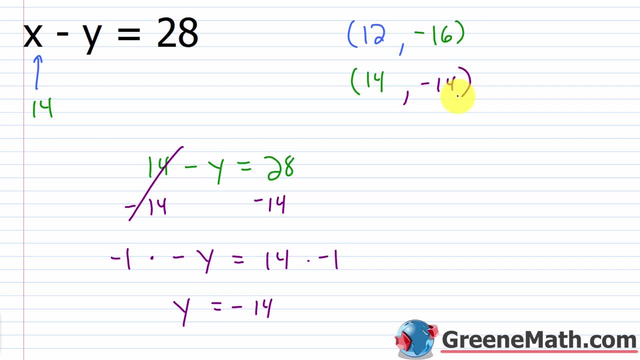 get y equals negative 14.. All right, so now let's plug in to the slope formula. So the slope formula again we have m is equal to y sub 2 minus y sub 1 over x sub 2 minus x sub 1.. 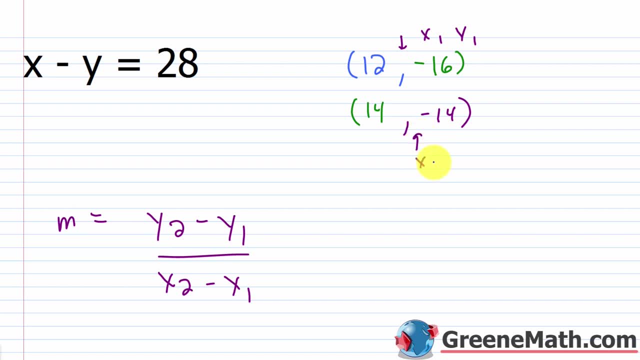 So let's just say this is x sub 1, y sub 1, and this is x sub 2, y sub 2.. So then, my y sub 2 is negative 14.. My y sub 1 is negative 16.. 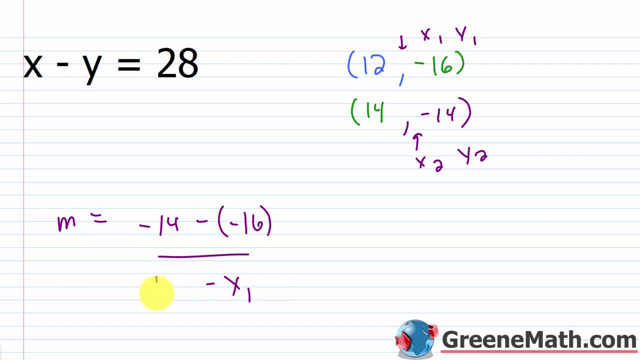 My x sub 2 is 14.. My x sub 1 is 12.. So negative 14 minus a negative 16 is the same thing as negative 14 plus 16.. So negative 14 plus 16 is going to give me 2.. 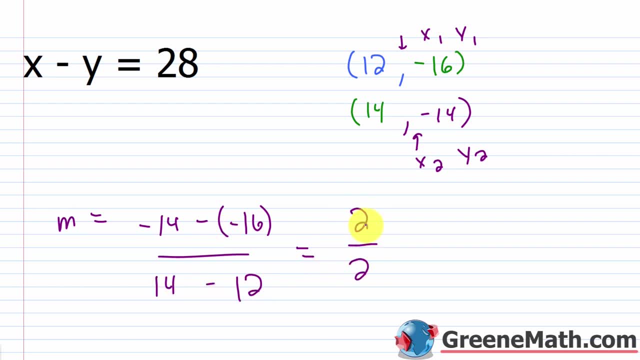 14 minus 12 is also 12.. So I'm going to plug in to the slope formula. So that's what I'm going to do: 2.. 2 over 2 is 1.. So you remember, when we solved this equation for y, we found that the slope was. 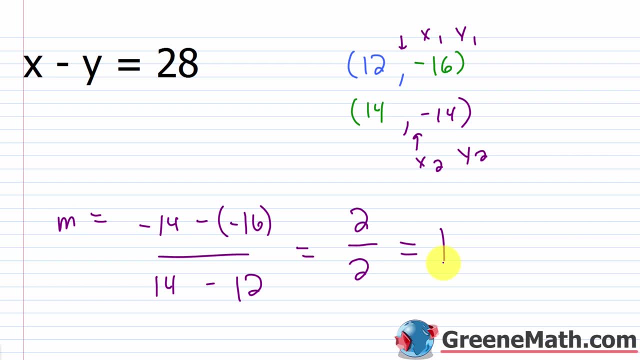 1. So look how much easier that was. This took us forever. We had to generate points, We had to plug it into the slope formula, you know, so on and so forth. So solving an equation for y is generally going to be the quickest way to find the slope. All right, let's look at one more of these. So 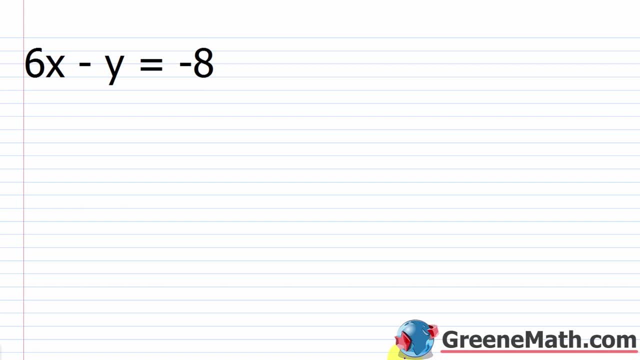 suppose you get 6x minus y equals negative 8.. Again you want to find the slope, Isolate y. on one side The slope is given as the coefficient of x. So let me subtract 6x away from each side of the equation. That'll cancel. You'll have negative. y is equal to negative 6x minus 8.. 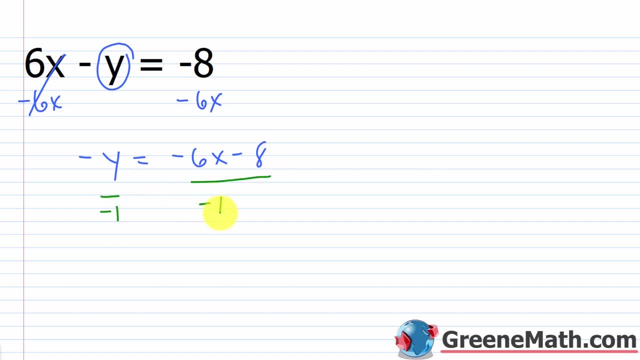 We would then just divide both sides by negative 1.. So I'd have: y is equal to negative 6x divided by negative 1 is 6x. Negative 8 divided by negative 1 is plus 8.. So then I have: y equals 6x. 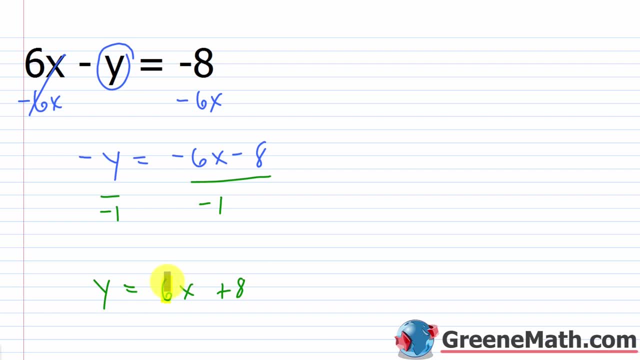 plus 8.. So the coefficient of y is equal to negative 6x divided by negative, 1 is plus 8.. The coefficient of x, which is 6, is my slope. This is m. All right, remember. y equals mx plus b. 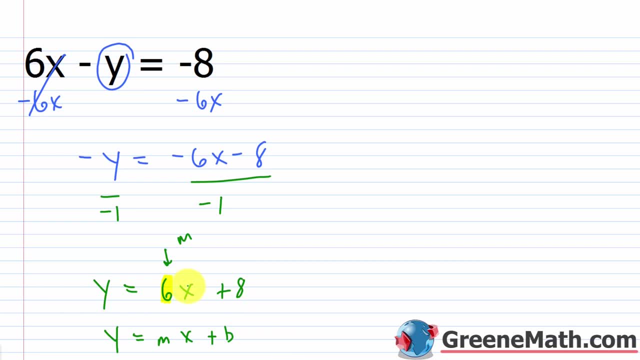 My y-intercept occurs at 0 comma 8. Again, plug in a 0 for x 6 times 0 would be 0. I'd have y equals 8.. So this is my y-intercept. And just one more time let me prove to you that this works. 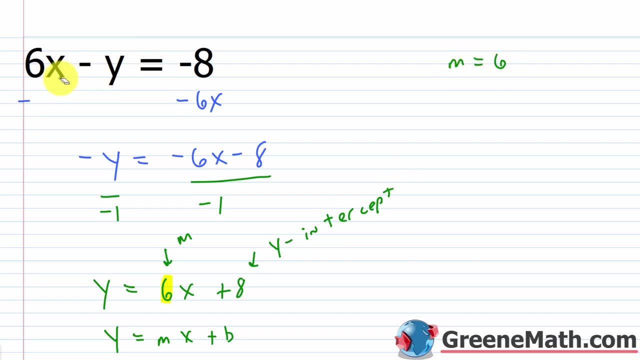 So I'm going to write here that m equals 6.. And I'll verify this for you. Let's just say that x was negative 0. So 6 times 0 minus y equals negative 8.. So this is: 0 minus y equals negative 8.. Divide: 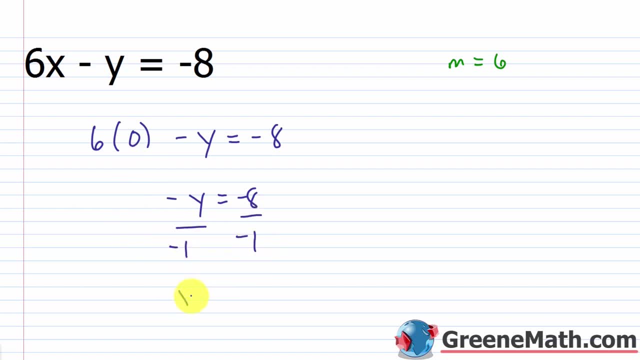 both sides by negative 1.. And I'll have: y is equal to 8.. So if x is 0, y is 8.. That's one point for us. As another point, let's say x was negative 2.. So negative 2 comma 1.. So 6 times negative 2 is. 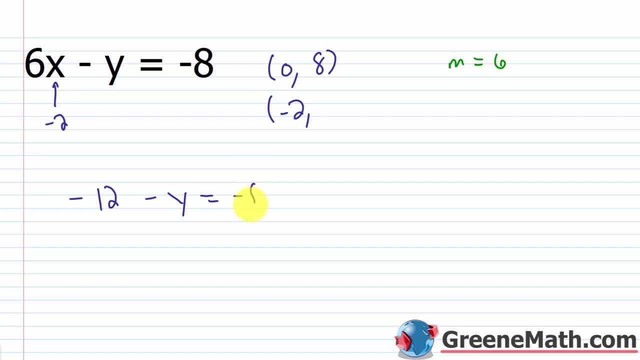 negative 12.. Then minus y equals negative 8.. So that's negative 2 comma 1.. So x times negative 2 is negative 8.. Let's add 12 to both sides of the equation. That'll cancel. I'll have negative. 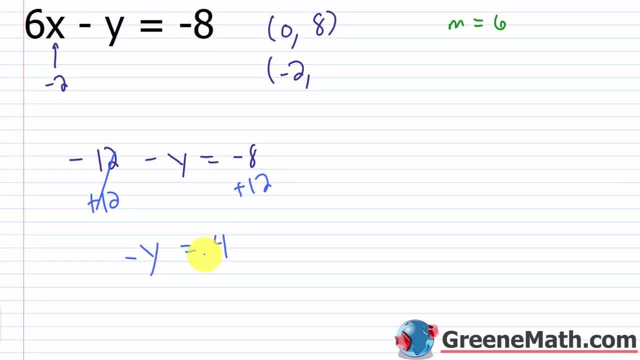 y is equal to negative. 8 plus 12 is going to give me 4.. Divide both sides by negative 1. You get y is equal to negative 4.. So again, let's use our slope formula now And we'll label each point arbitrarily. Let's say: this is x sub 1, y sub 1.. This is x sub 2, y sub. 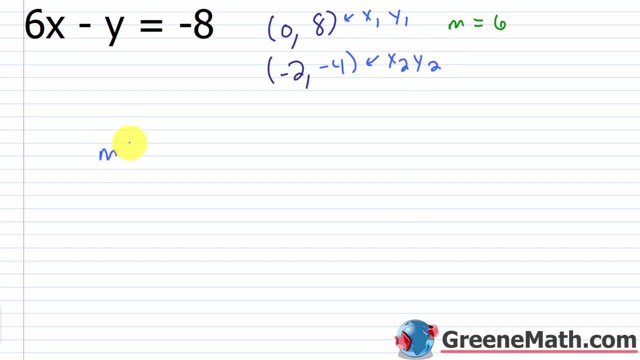 2. So I use my formula: m equals y sub 2,, which is negative 4, minus y sub 1,, which is 8, over x sub 2,, which is negative 2, minus x sub 1,, which is 0.. So negative 4 minus 8. 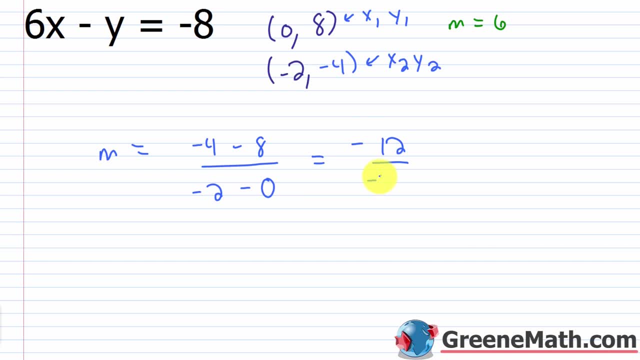 is negative 12, over negative 2 minus 0,, which is just negative 2.. And if I divide negative 12 by negative 2, negative over negative is positive. 12 divided by 2 is 6.. So I get m. 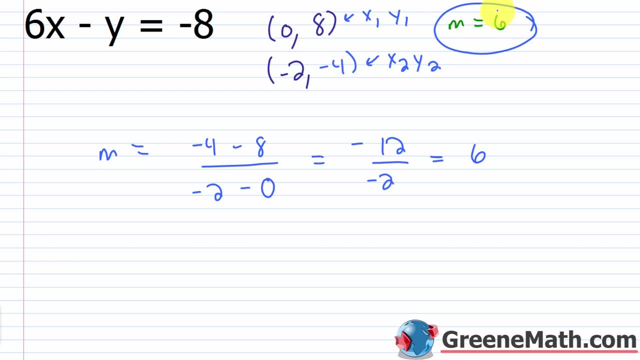 equals 6 in the end, which is 4.. This is what I found pretty quickly by just solving the equation for y. So kind of some wrap-up notes here. Finding slope is not very difficult at all. You can use the slope formula. 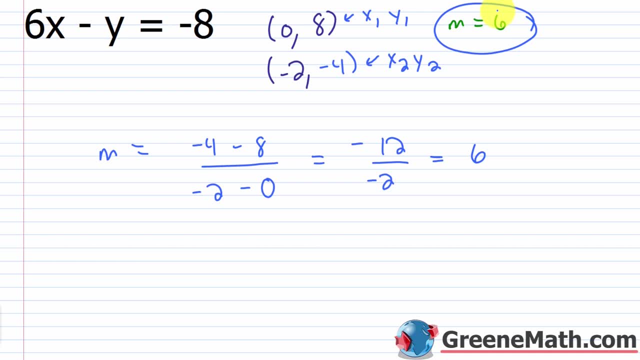 if you know two points on the line. So if you're given an equation and you want to use the slope formula, generate two points for the line and plug them into the slope formula. Otherwise, if you want to find the slope, you can solve the equation for y, The slope. 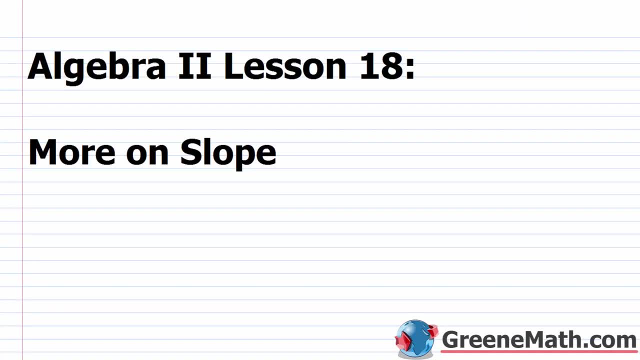 is given by the coefficient of y. Hello and welcome to Algebra 2, Lesson 18.. In this video we're going to continue to learn about slope. So in our last lesson we talked all about how to find the slope of a line. 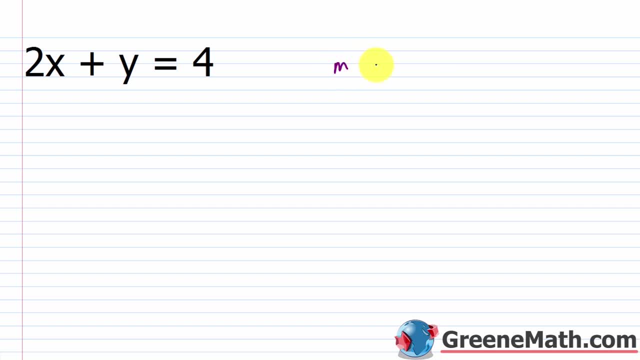 And we learned the slope formula, which was m, which denotes slope is equal to y sub 2 minus y sub 1 over x sub 2 minus x sub 1.. So we learned this formula. So if I had an equation, for example, like this one: 2x plus y equals 2x plus 2x plus y equals 2x plus y. 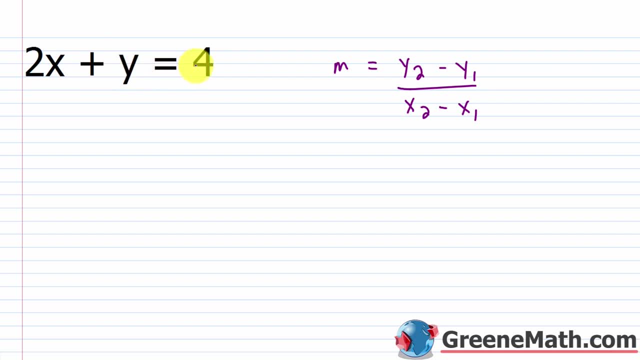 4, I could find two points. I could plug those two points into this formula and I could calculate a slope. So let's do that real fast. So for this one two points. if I choose 0 for x, my y-intercept, I would have 0 times 2, so this would go away. I just have y equals 4.. 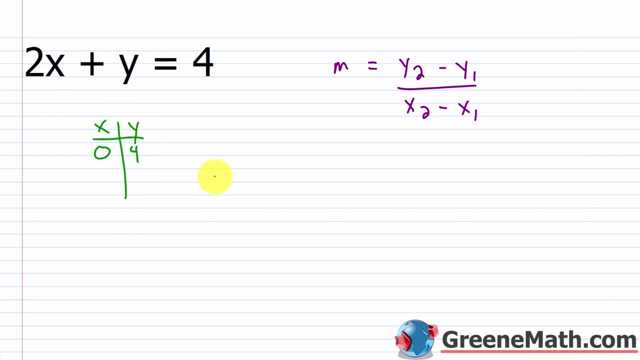 If I chose 0 for y, I would have 2x is equal to 4,. I would divide both sides by 2, and we'll get x equals 2.. So the x-intercept occurs when y is 0, and x is 2.. So I have. 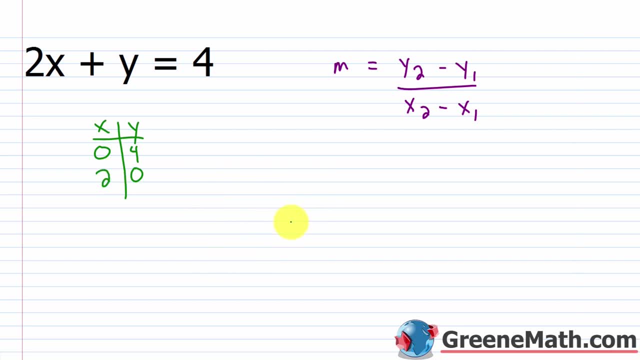 two points there. Once I have my two points, I label them so they're ordered pairs: one is 0 comma 4, the other is 2 comma 0. So again, it doesn't matter which I label as which. 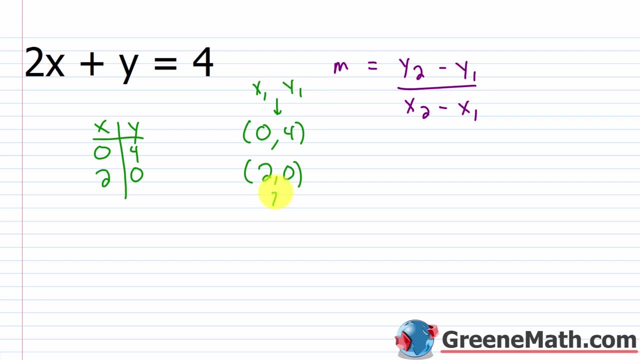 I'm going to label this one as x sub 1, y sub 1, and this one has x sub 2, y sub 2. you could switch that around and you're going to get the same answer. So I plug into this formula: I have m is equal to. for y sub 2, I have 0 minus. 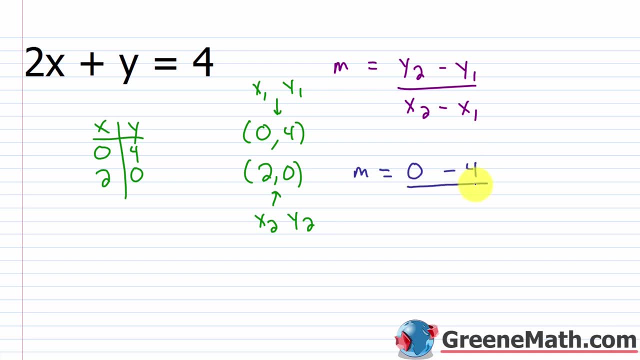 for y sub 1, I have 4 and this is over. for x sub 2, I have 2 minus. for x sub 1, I have 0. So 0 minus 4 is negative 4. 2 minus 0 is 2 negative. 4 over 2 is negative 2. so my slope m. 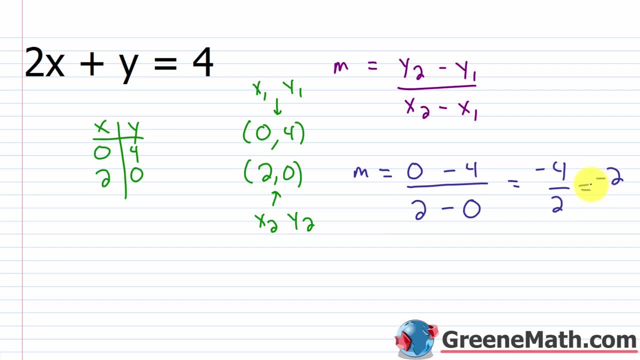 is negative 2.. So we're going to talk more about what that means in a second, but I want to show you something else. we talked about this in the lesson also. The quicker way to kind of get the slope is to solve the equation for y. We put it into a format that is known as slope intercept. 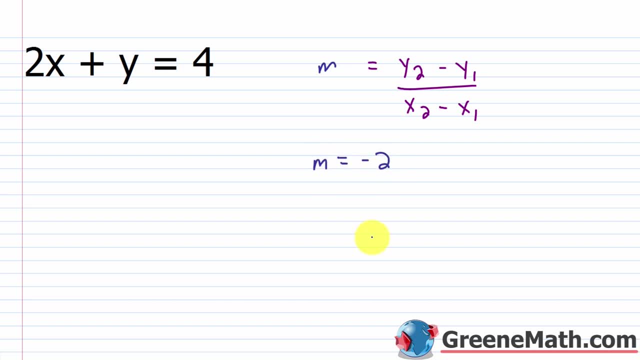 form. So let me just note that m is equal to negative 2 here. So slope intercept form looks like this: it's y equals m, which is your slope times x plus b. So this is slope intercept form, and if you haven't gotten to this in your class yet, you're going to cover this. 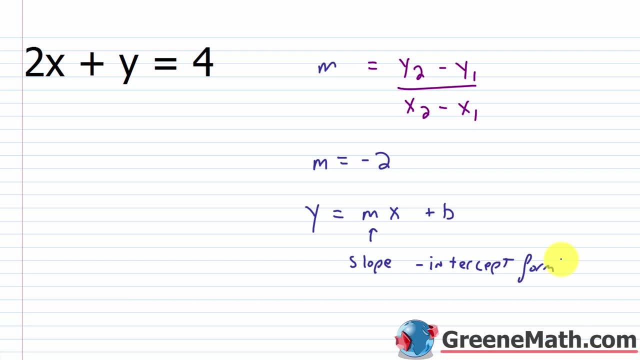 when you talk about different forms of the line. okay, But it's good to kind of get started with it now, because it's just a quick and easy way to get started. So let's get started. So if I solve this for y, meaning I isolate y on one side of the equation by itself, I just subtract. 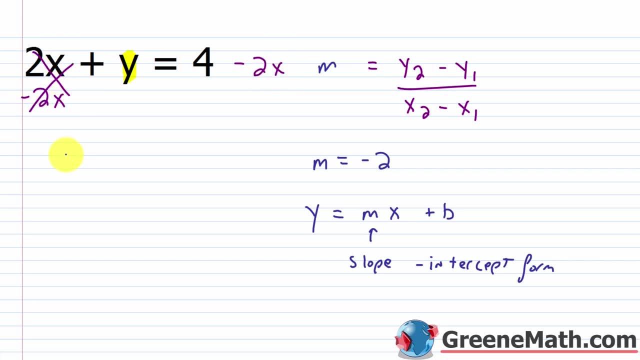 2x away from each side. This will cancel. I'll have: y is equal to negative, 2x plus 4.. Now again, it's y equals m, the slope times x plus b. So y equals negative 2.. Negative 2 is m. This is the. 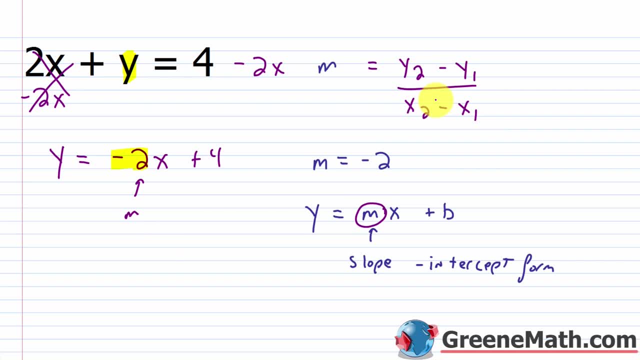 slope. We found that over here by doing a more complex equation, So we're going to do a more complex procedure, right? We had to generate points, We had to label the points, We had to plug them in. you know so on and so forth. This is so much faster. All I got to do is solve for y. 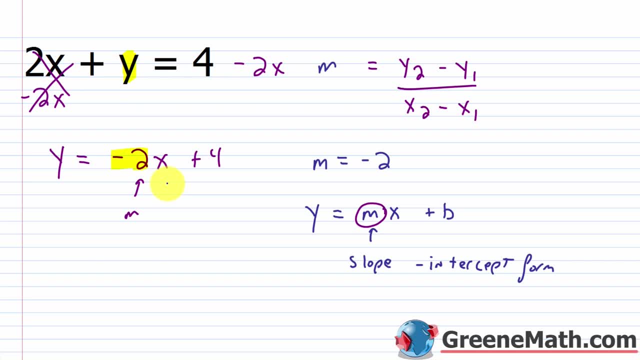 and look at the coefficient for x. So it's kind of an upgraded procedure. So we solve the equation for y. We automatically know the slope. Now the other thing we have is we have the y intercept. Remember to get the y intercept. I plug in a 0 for x. 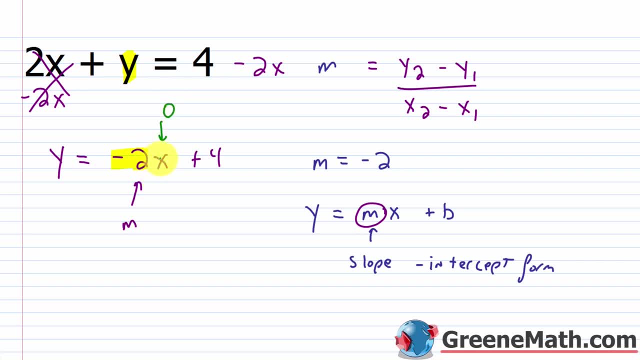 And I find out what y is. Well, if I plug in a 0 for x, I'm always going to have this right here. right, because 0 times m would give me 0. So this would cancel away and I'd have a y intercept that. 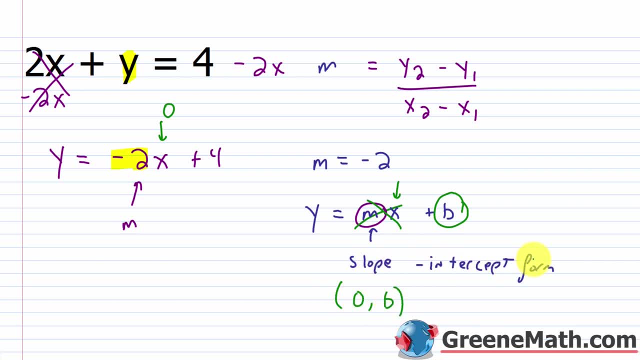 occurs at 0 comma b. That's why it's called slope intercept form. We know the slope and we know the y intercept, All right. so for this particular one, I know that the y intercept would occur at 0 comma 4.. Now, what can I do with this information? 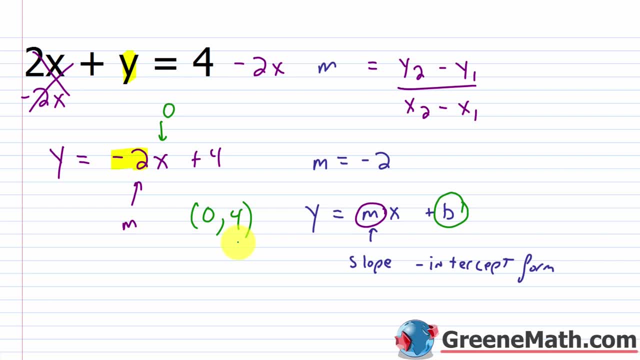 Well, again, it allows us to know the slope very quickly, It allows us to know the y intercept very quickly, But it also allows me to graph very, very quickly. I don't have to sit there and generate three points and then go plot the points and do all this work. I can simply take this point. 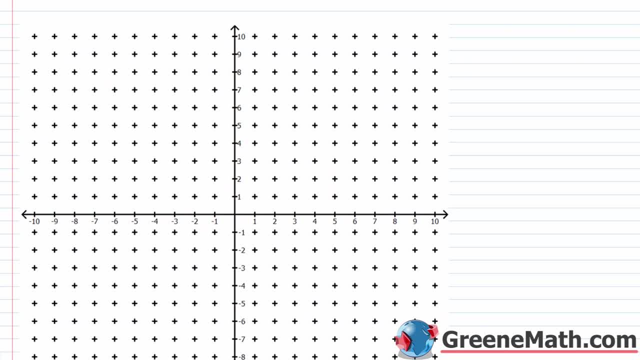 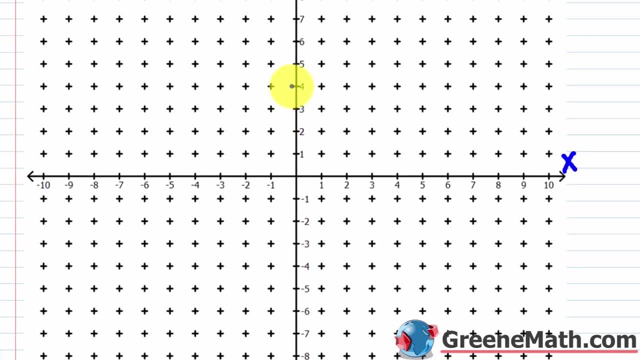 right here: 0 comma 4.. I can go to my coordinate plane and let me label this: This is the x axis, This is the y axis. So where's 0 comma 4?? Well, that's going to be right here. Now, remember my. 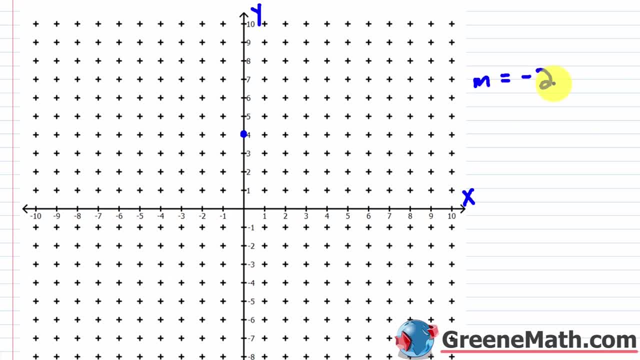 y is equal to negative 2.. So what does that mean? We talked about that in the last lesson. We talked about rise over run. So rise over run. here is negative 2 over 1, right, because I could take negative 2 and just put it over 1.. So I rise, negative 2.. That means I just fall, So I'm going. 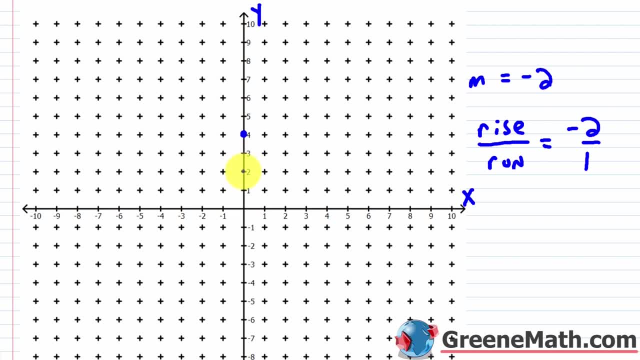 to go down two units. I run 1. That means I go to the right one. So when we talk about running, we're talking about horizontal movement. So if that's positive, I'm going to the right, If it's negative, I'm going to the left. When we talk 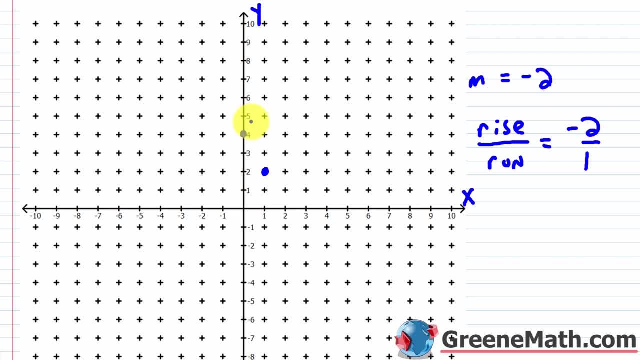 about rising: if it's positive, I'm going up, If it's negative, I'm going down. So that's why negative 2 over 1. I went down 2 to the right 1.. And just do that again. So down, 2 to the right, 1.. And now: 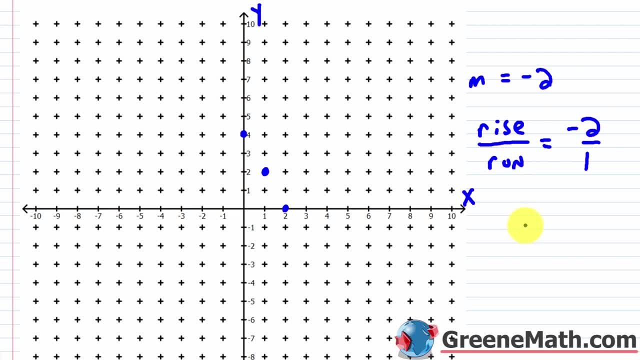 I have three points here. Of course, I only need two to make a line, but it's nice to have three. I'm going to go ahead and just draw my line. And this is the graph. the equation 2x plus y is equal to 4.. Now look how fast I found the slope. look how fast I found the. 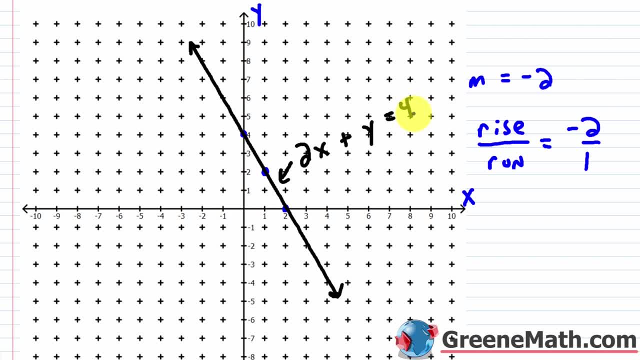 y-intercept and look how fast I graphed this thing. You know, in the previous lessons we sat there and we generated points and we, you know, we did all these complex procedures- or not really complex, just kind of tedious things. Now, if I just solve this equation for y, I can go to my coordinate. 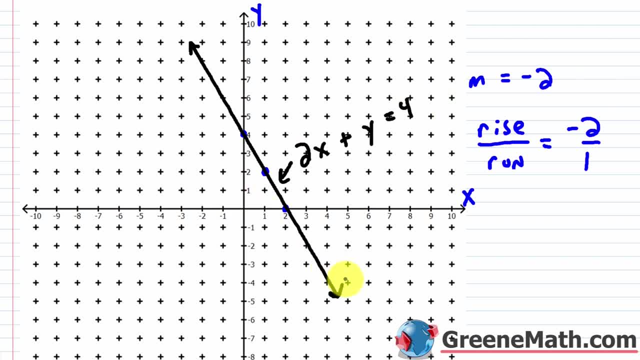 plane and graph it in like two seconds. Okay, so this is the fastest way to graph a linear equation in two variables. Just solve it for y, use the y-intercept as your first point and then use your slope to generate one or two or even three more points so that you can sketch the graph. All right. 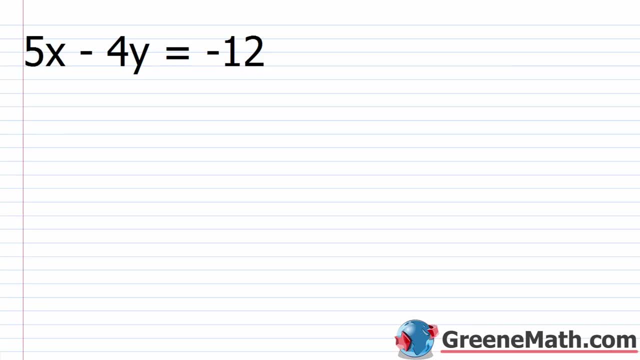 let's take a look at another example. So let's say you saw 5x minus 4y equals negative 12 and I asked you to find the slope, find the y-intercept and to graph it. Okay, it's a common. 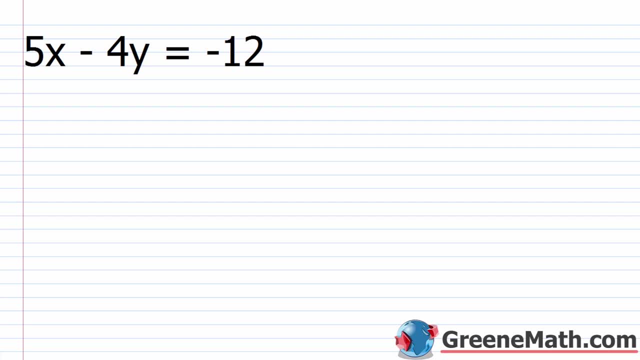 example that you might see. So let's start out by solving this for y. So this is y here. We've got to get it by itself. So my first objective is to move this over here, and I do that by just subtracting 5x from both sides of the equation, So this would cancel itself out. I'd 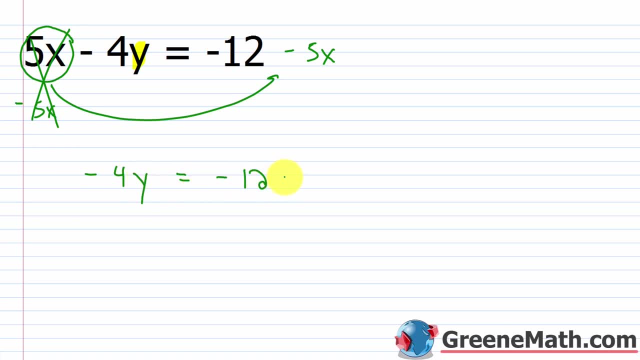 have negative 4y is equal to negative 12 minus 5x. Of course I'm going to switch the order there. I'm just going to write that as minus 5x, minus 12.. And now to get y by itself, all I need to do is divide. 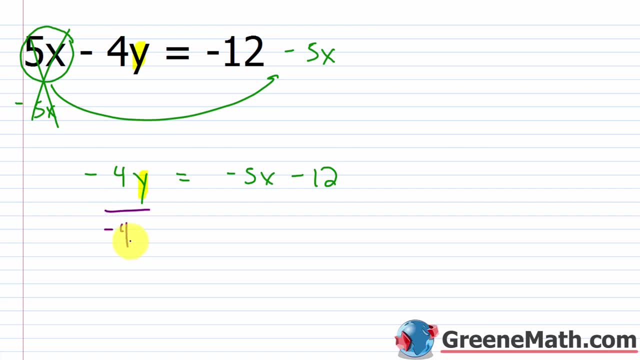 both sides of the equation. So I'm just going to write that as minus 5x minus 12.. And now to get y by itself, all I need to do is divide both sides of the equation by negative 4.. So I'm going to divide this side by negative 4, and I'm going to divide this side by 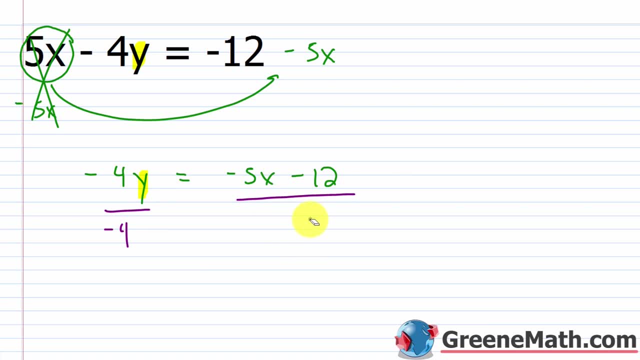 negative 4, but I'm going to do it to where I split it up. So what I mean by that is I'm going to put negative 5x over negative 4, and then I'm going to space this out and put plus negative 12 over. 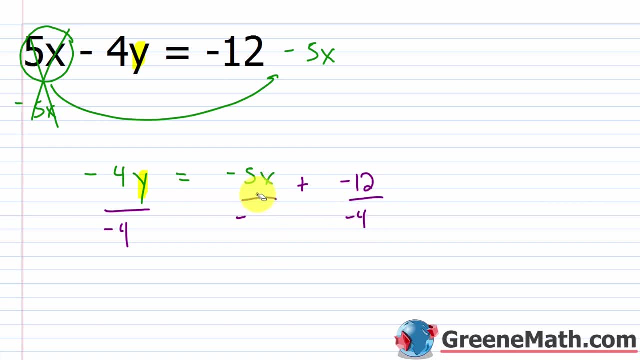 negative 4.. So that's going to make it obvious what I need to simplify to here. This will cancel with this and I have y And this equals negative 5 over negative 4.. Can't really do anything with that, But I'm going to write 5 fourths, because I know the negative over negative will be positive, So 5. 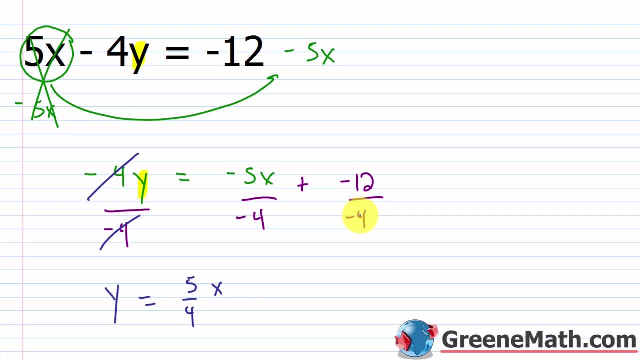 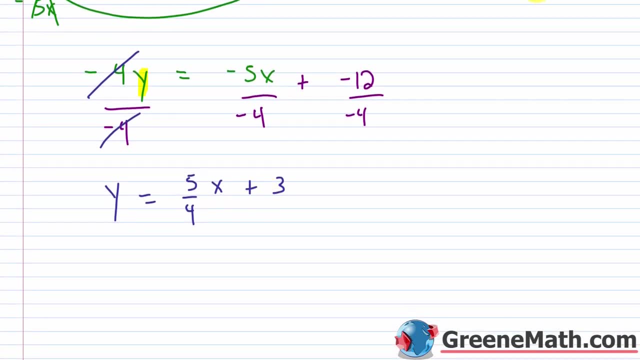 fourths x, and then negative 12 over negative 4, I can write that as 3.. So plus 3.. Now, what information do I have? Well, I have my slope. Remember it's y equals m, the slope times x plus. 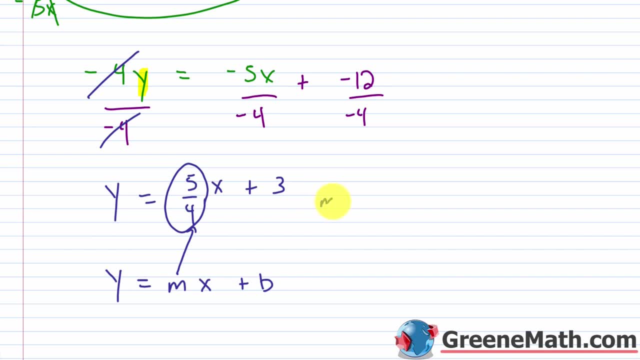 b. So my slope is 5 fourths m equals 5 fourths. Now b again. if I think about the y intercept, it occurs at 0 comma b. Well, b is 3.. So the y intercept will occur at 0 comma 3.. So let's use: 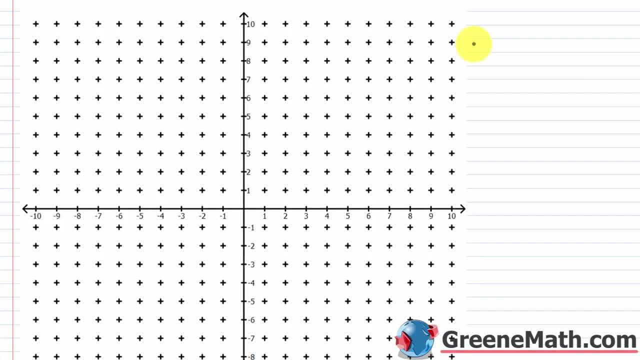 this information to graph the equation. So again we found that this was y equals 5 fourths times x plus 3.. Now my y intercept occurs at 0 comma 3.. So 0, comma 3.. And again, slope m is 5 fourths. So where is 0 comma 3?? Well, it's going to be right. 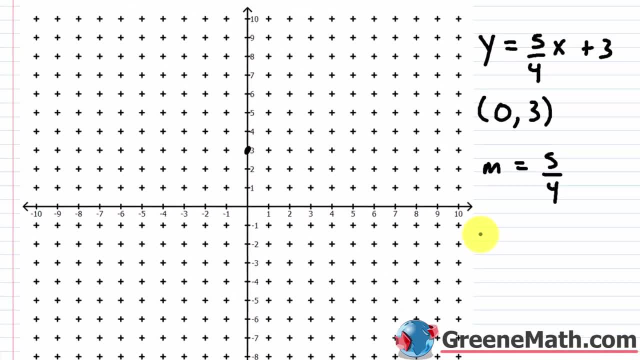 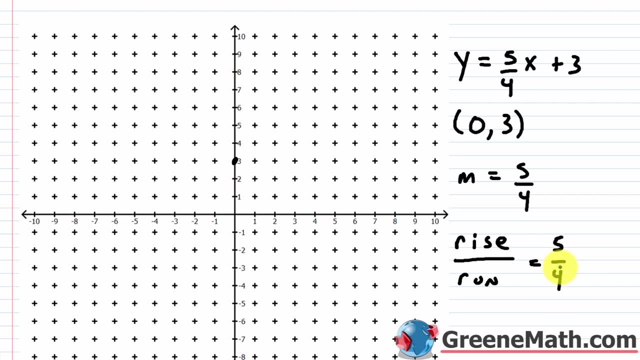 here Now for a slope of 5 fourths again you think about. rise over run is equal to 5 over 4.. And it's very, very easy to figure out what's going on here. If rise is 5, that means I just 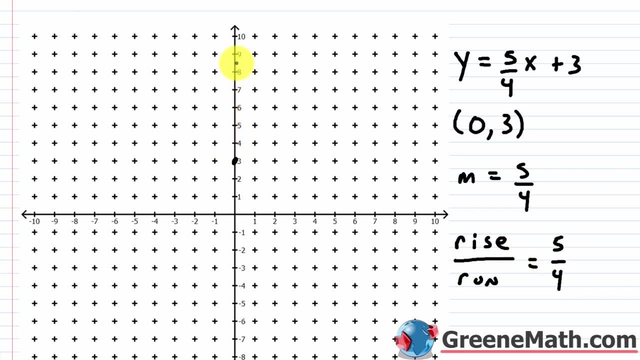 go up 5 units, So 1,, 2,, 3,, 4, 5.. Now, if run is 4,, then I can just go up 5 units, So 1,, 2,, 3,, 4, 5.. 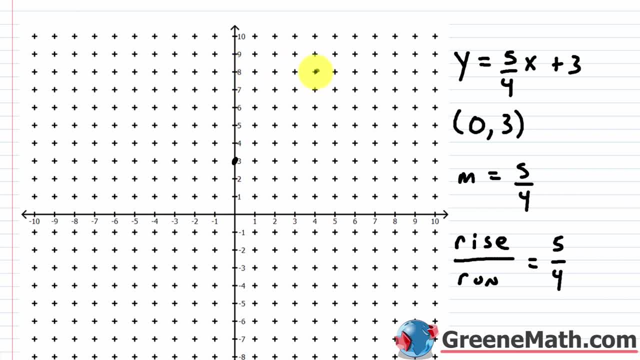 And I go to the right: 4.. 1,, 2,, 3, 4.. That's a point right there And you can check that by plugging it in. So that's an x value of 4, a y value of 8.. So if I plugged in a 4 here, 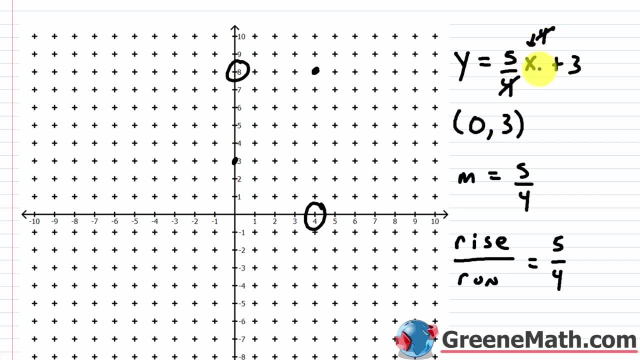 5 fourths times 4, you know the 4s would cancel. You'd have 5 plus 3, which is 8.. So that works out mathematically All right. So now that we see that, can I rise 5 and go to the right 4? 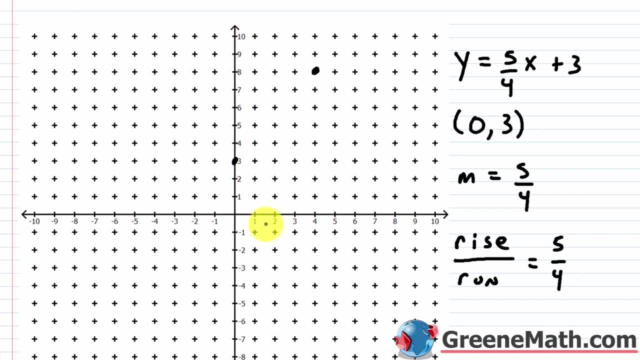 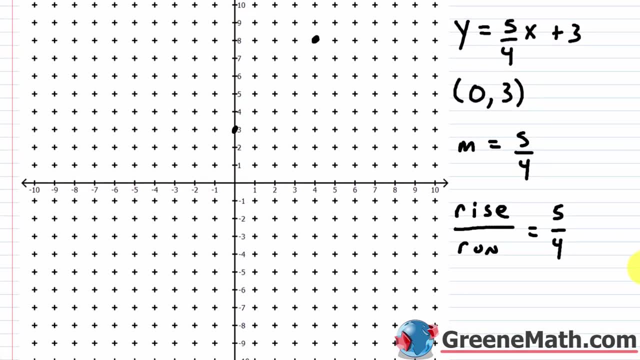 using what I have here, No Run off. So what I want to do is I want to use a little trick, And you'll probably have to do this depending on the scale of what you're using to create your graph. But 5 over 4, realize, with. 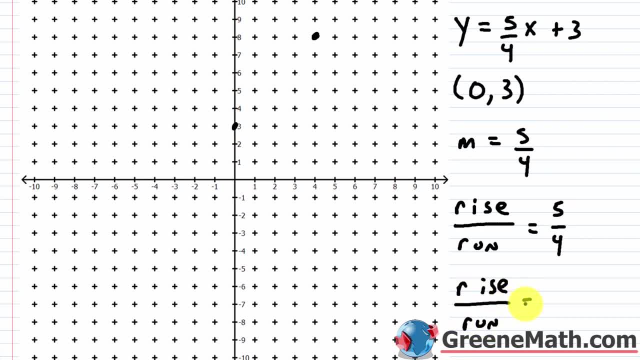 fractions. I can write this as negative 5 over negative 4.. Negative over negative is positive, So the value of that fraction is still positive And I can use that trick to start here And I can say: well, the rise is negative 5.. So I'm going to go. 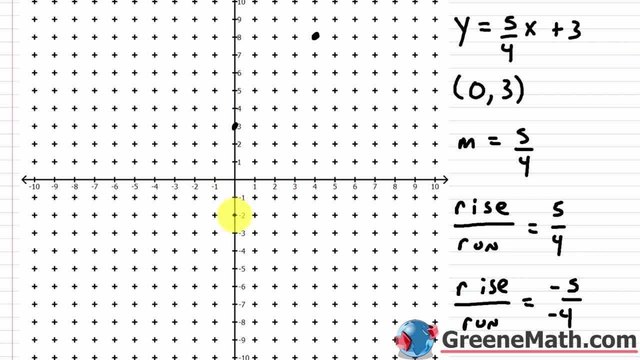 1,, 2,, 3,, 4,, 5 down, The run is negative 4.. So horizontally, a negative 4 means I'm going to the left. So go to left 1,, 2,, 3,, 4.. And that's where I'd be. And if you start at this point, 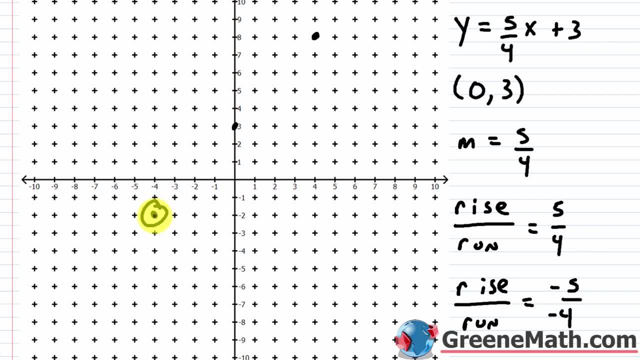 you can use this. to get back to this. I'd go up 1,, 2,, 3,, 4, 5.. Go to the right: 1,, 2,, 3,, 4.. So you can go back and forth in how you do that. So if you have a positive value, 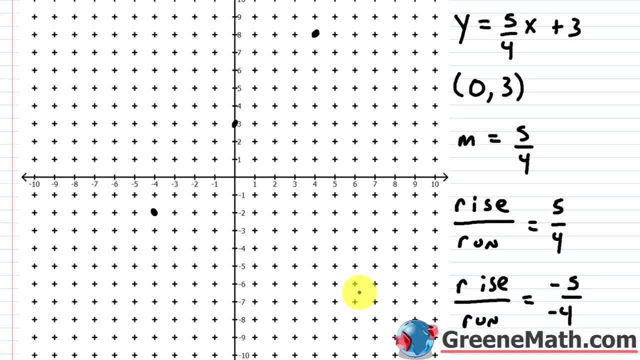 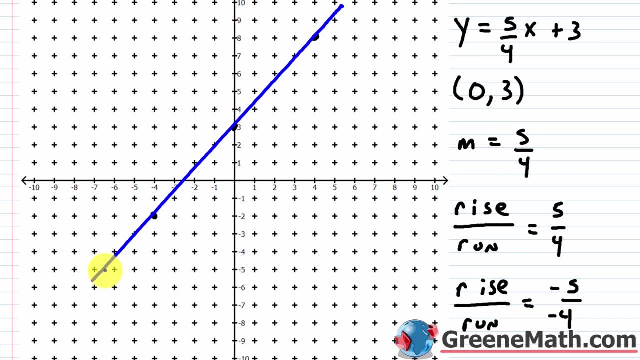 you can go negative over negative to get another point if you need to do that. So now that we have three points here, let's go ahead and sketch our graph. OK, And let me just label this. Originally we had it as 5x minus 4y equals negative 12.. 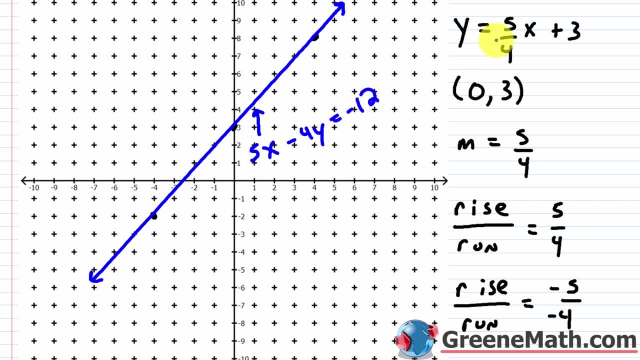 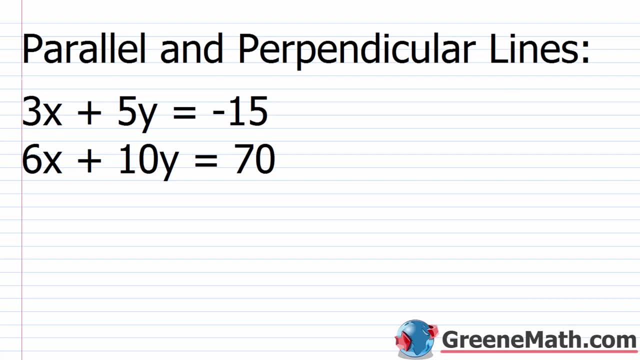 You could also label it with: y equals 5,, 4 is x plus 3.. It doesn't really matter, You're just saying: hey, this is the equation for this line that we just graphed. All right, So now that we understand how to kind of manipulate an equation. 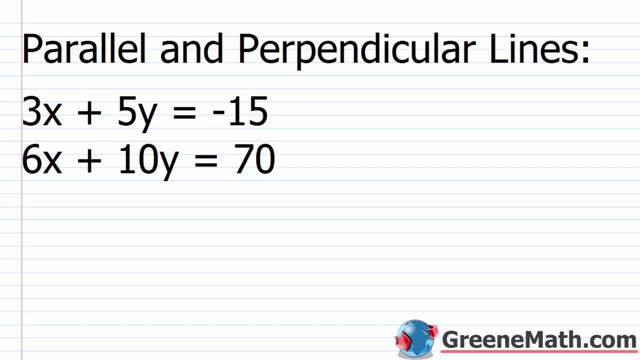 and we can now graph very quickly. we can now find slope very fast. let's talk about something that's going to come up usually in the next section. So I want to talk about parallel and perpendicular lines, So two non-vertical lines that have the 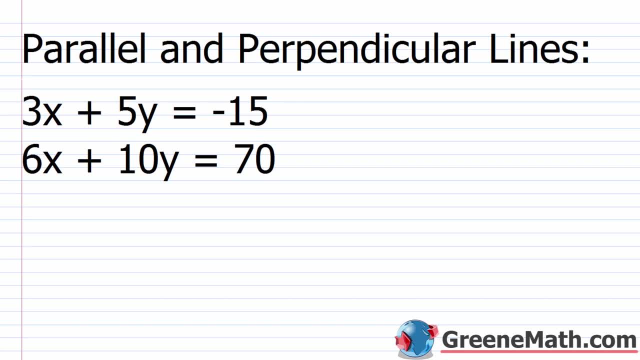 same slope are parallel, So you'll know that they have the same slope. if you solve each equation for y, You'll have the same slope but a different slope. So you'll know that they have the same slope. if you solve each equation for y, You'll have the same slope but a different slope. So you'll know. 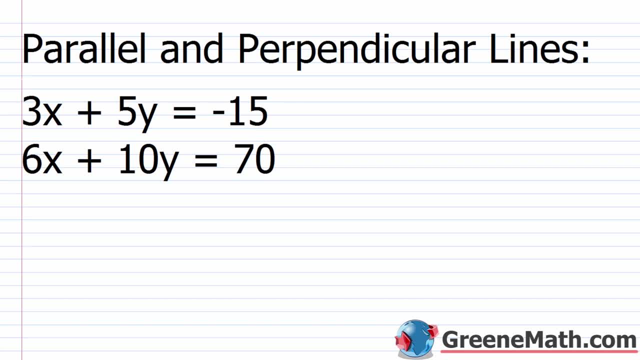 different y-intercept. those are parallel lines And I'll graph an example of that so you can see what that looks like. Now, two perpendicular lines. okay, perpendicular lines have slopes whose product is negative 1. So, again for that, you would just solve each equation. for y, You'd. 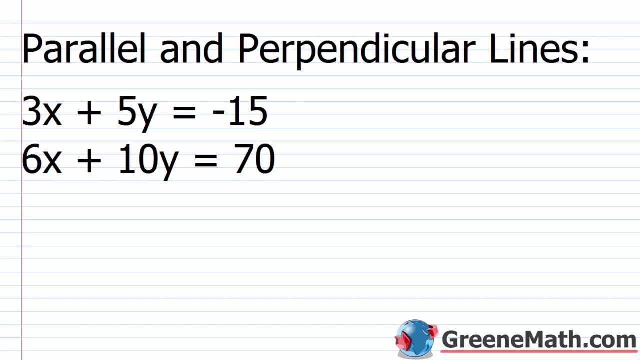 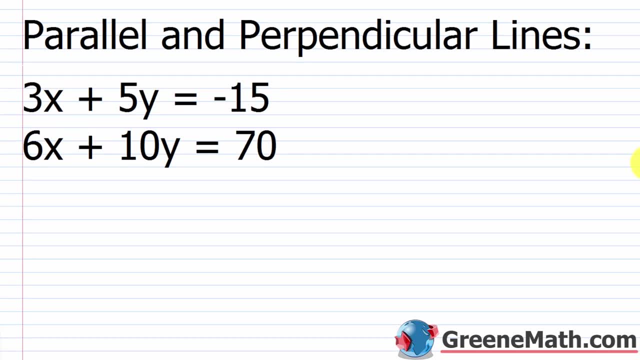 look at the slopes and you'd see if you multiply them together. if you get negative 1, those two lines are going to be perpendicular. So very, very easy topic overall. Okay, let's go ahead and take a look at the first problem. 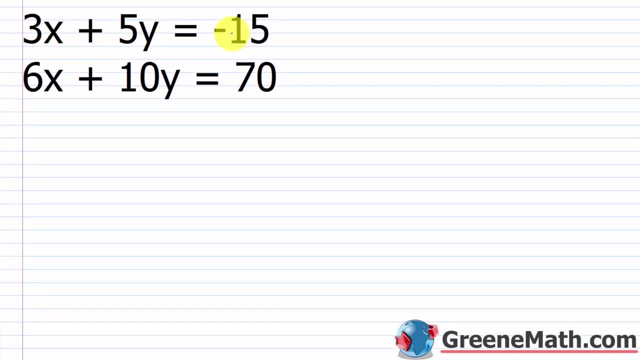 So we have: 3x plus 5y equals negative 15, along with 6x plus 10y equals 70. So the smart way to attack this problem is to solve each equation for y. We want it in the format of: y equals m, the slope. 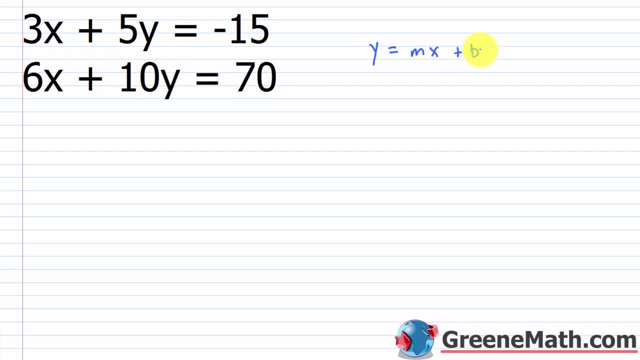 times x plus b, the y-intercept. Again, I can't say this enough- this is called slope-intercept form. So when we solve this for y, we're going to have a slope-intercept form. So we're going to have: 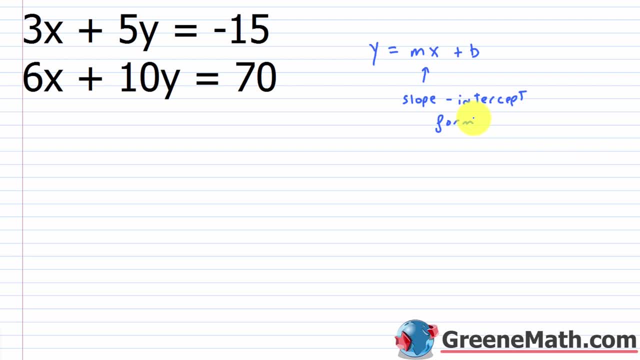 a slope-intercept for y, We will know the slope of each equation. We can then look at those two slopes and we can see if they're the same. If they're the same, we have parallel lines. If they're different, then we're going to check to see if the product of those two slopes would be. 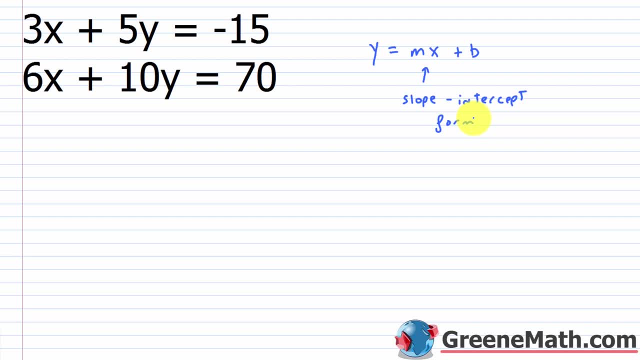 negative: 1. If that's the case, we have perpendicular lines, And in some cases we're not going to have parallel lines or perpendicular lines. You'll see problems where they're just neither All right. so let's solve the first one for y here. So 3x plus 5y equals m, the slope times. 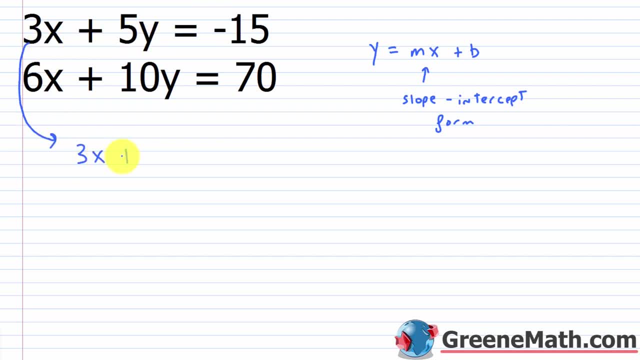 y equals negative 15.. So 3x plus 5y equals negative 15.. If I want to isolate y, then what I'm going to do is I'm going to start by subtracting 3x away from each side of the equation. So that's. 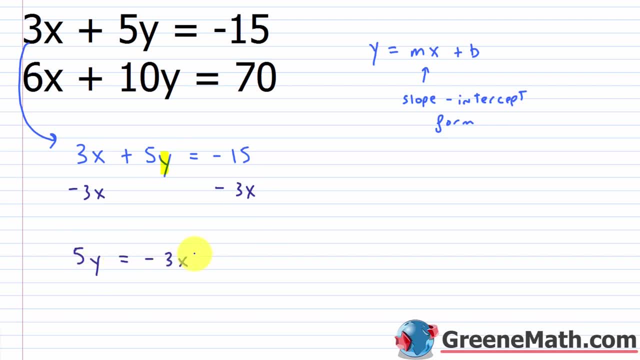 going to give me. 5y is equal to negative 3x minus 15.. Then I'm going to divide each side of the equation by 5. And what's that going to give me? Well, we know that this would cancel with this. 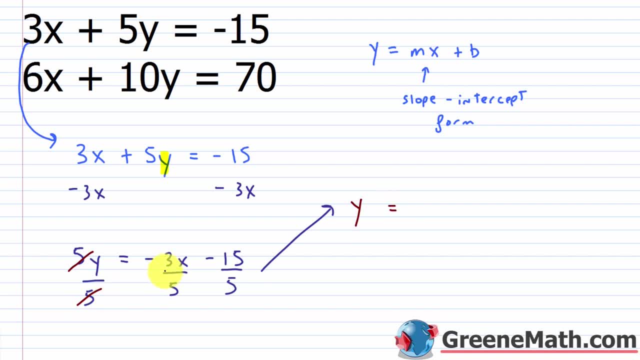 So y is equal to negative 15.. So we're going to divide each side of the equation by 5. So y is equal to: I'll have negative 3 fifths x. So negative 3 fifths x And then minus. we have 15. 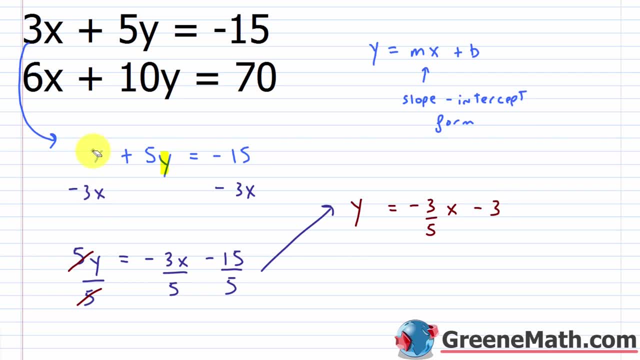 over 5,, which is 3.. So let's erase this, And I'm just going to drag this over here. Okay, let's take a look at this one now. So 6x plus 10y equals 70. So again, 6x plus 10y is equal to 70.. To solve: 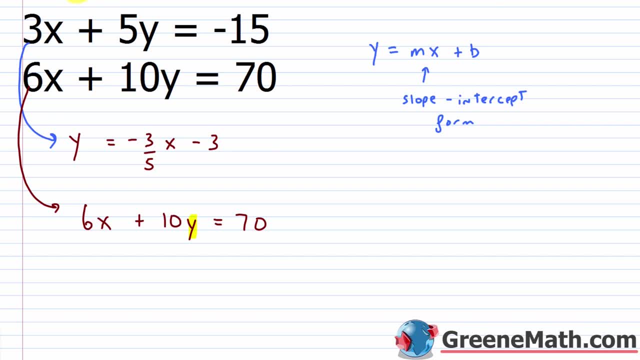 this: I'm going to subtract 6x away from each side of the equation, So that's going to give me 10y is equal to negative 6x plus 70.. I want y by itself, So let's divide both sides of the equation. 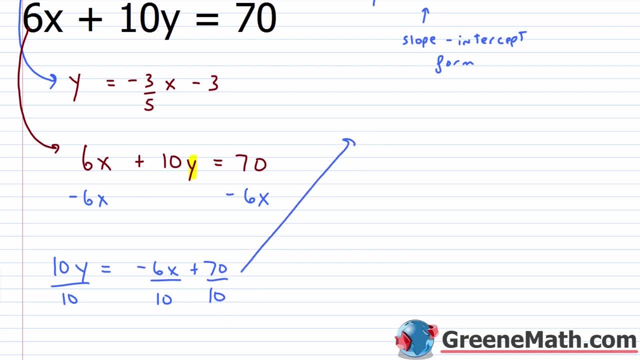 by 10. And I'll do that over here, So there's room. So this cancels with this. Y is by itself and it's equal to negative 6 over 10.. Well, we know that they're both divisible by 2. So 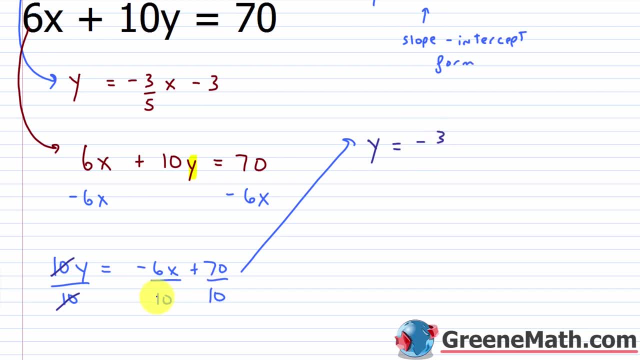 it's going to be negative. 6 divided by 2 is 3.. 10 divided by 2 is 5.. So this is negative. 3 fifths, then times x, then plus We have 70 over 10, which is just 7.. So let's erase this. 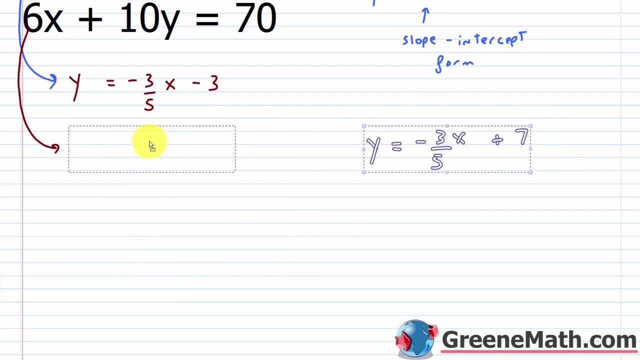 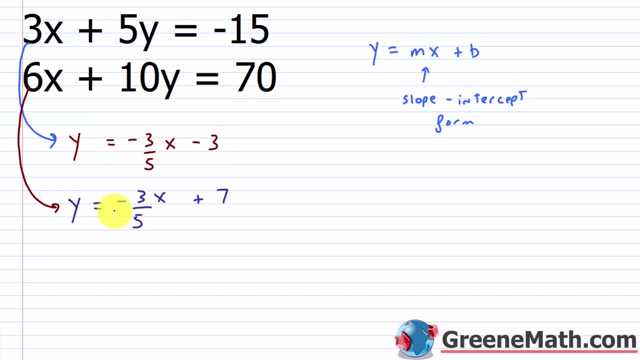 And let me drag this guy over here now. So we see that we have: y equals negative 3 fifths, x minus 3, and y equals negative 3 fifths x plus 7.. So what can we conclude here? We can see that the slope here is negative 3 fifths and the slope here is also negative 3. 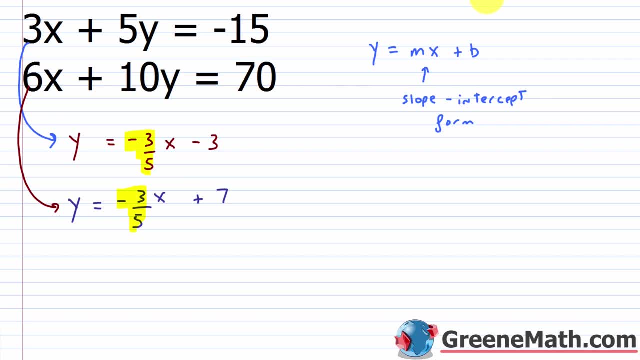 fifths. So when two lines have the same slope and they have different y-intercepts. this one would have a y-intercept that occurs at 0 comma negative 3. This one would have a y-intercept that occurs at 0 comma 7.. These two lines are parallel, right, They are parallel lines. 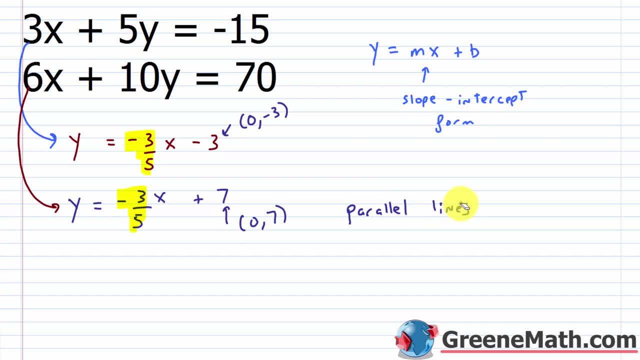 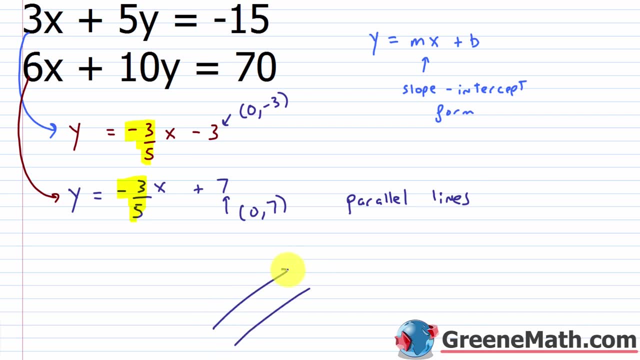 And let me make these ease a little better. What are parallel lines? Well, essentially it looks something like this, And I know I didn't draw that perfectly- but parallel lines will have the same amount of distance between them, no matter how far out you go. So you can imagine a coordinate plane. just stretch it in your head. 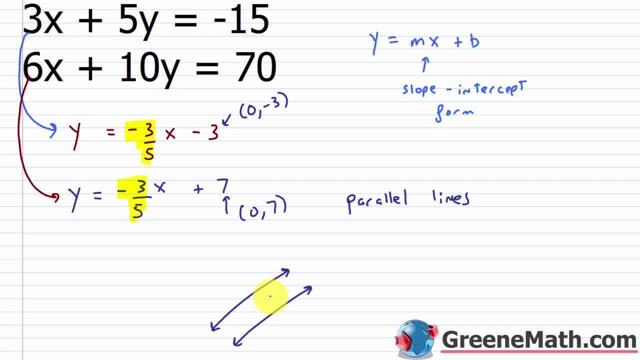 forever and ever and ever. These two lines have the same slope, the same steepness, So they have the same distance between them, always. They're never, ever, ever going to intersect or touch each other in any way. So let's go ahead and take these two down to the coordinate plane. We're going to graph them. 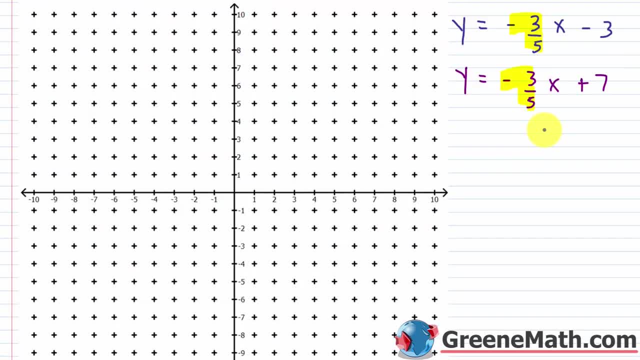 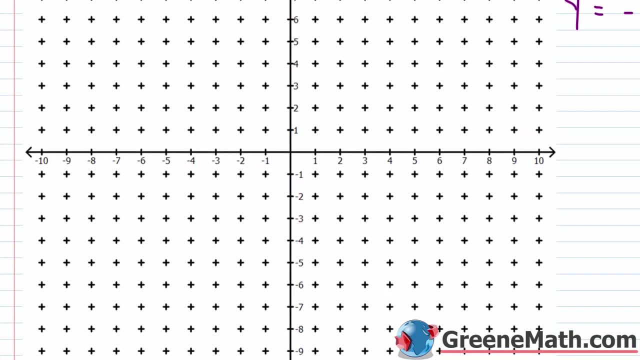 and we're going to take a look at what parallel lines would look like. All right, so for the first equation, y equals negative 3, fifths x minus 3. The y-intercept occurs at 0 comma, negative 3.. So that's right here. And then the slope. 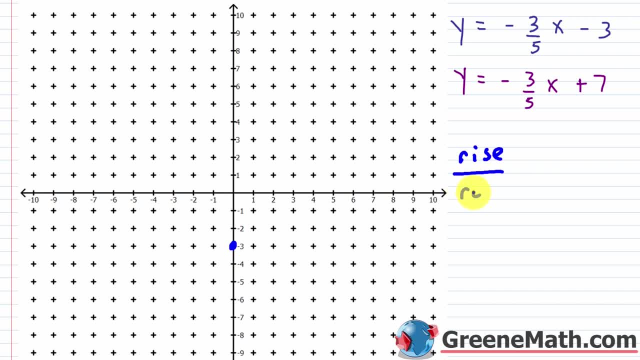 again, rise over run is equal to negative 3 over 5.. So I can rise negative 3 and run 5, or I can rise 3 and run negative 5.. Remember, negative over positive is the same as positive over negative. So again, these are little techniques you can use to get points, depending. 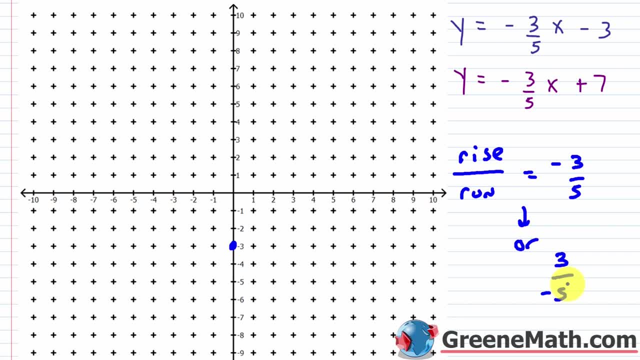 on what the scale of your coordinate plane is. So I'm going to go with a negative 3 over 5.. So I would go down 3, 1,, 2, 3, to the right, 5.. 1,, 2,, 3,, 4,, 5.. There's a point Now. let's say I want to 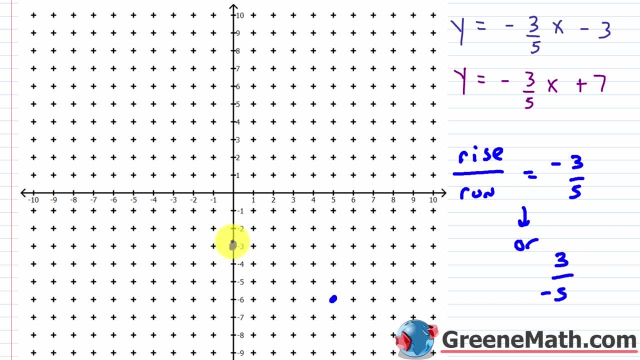 make a point somewhere over here, So let's use this one. Let's go up 3.. 1,, 2,, 3.. We're going to go to the left: 5.. 1,, 2,, 3,, 4,, 5.. 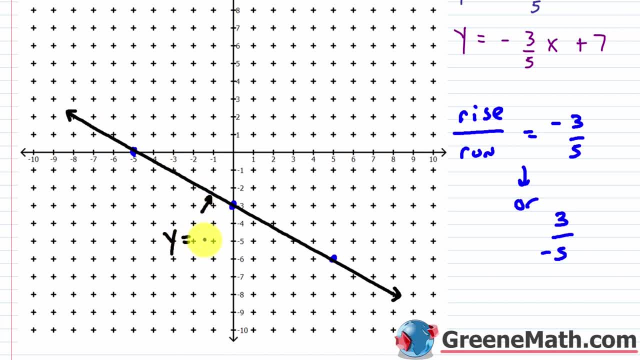 OK, and again this is: y equals negative 3 fifths x minus 3.. Or again you could also write: 3x plus 5y equals negative 15,. whatever you want to write, All right. for the next one, we have y equals. 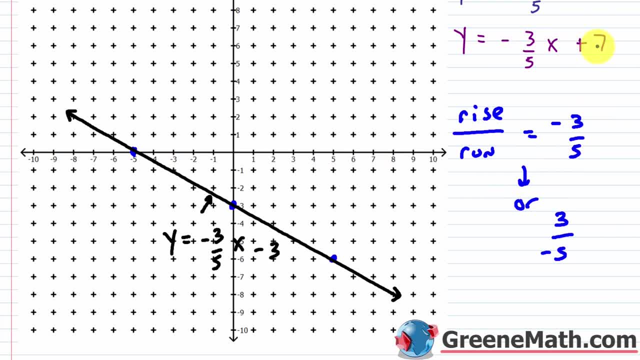 negative: 3 fifths x minus 3.. So we're going to go up 3, 1,, 2,, 3,, 4,, 5.. And again this is y equals x plus 7.. So same slope, different y-intercept. Y-intercept there is at 0, 7.. My slope is again: 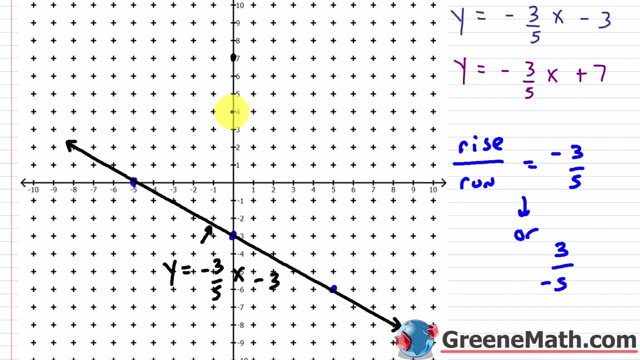 negative: 3 fifths. So again, I'm going to go down 1,, 2,, 3, to the right: 1,, 2,, 3,, 4,, 5.. And I'll just do that. again, Let's go down 1,, 2,, 3, to the right: 1,, 2,, 3,, 4, 5.. OK, let's go ahead. 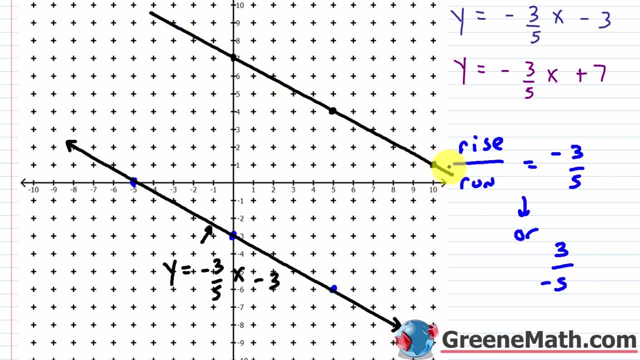 and graph this. OK, and let me label this. This one has: y equals negative 3 fifths x plus 7.. And again you could write that as: 6x plus 10y equals 70. It's the same thing. in the end, right 1 is solved for y 1 is not. So now that we have 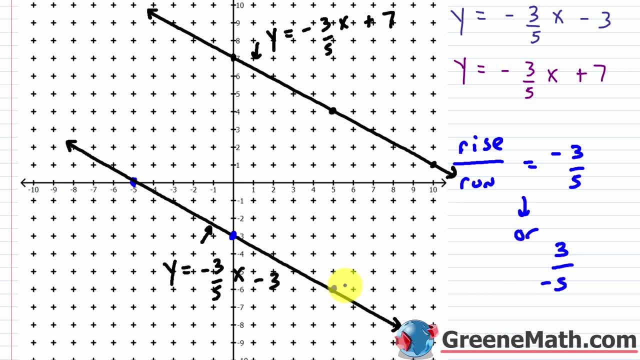 this drawn, we can observe what parallel lines look like. There are two lines that will never, ever intersect on the coordinate plane right. These are parallel lines And again you can see that they have the same slope or the same steepness. OK, But they have different y-intercepts, So they're in different. 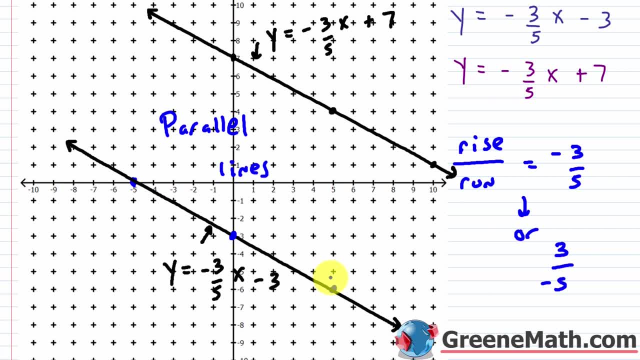 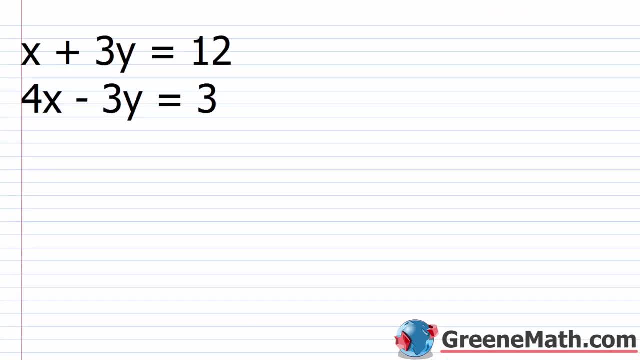 locations of the coordinate plane And again, they're never, ever ever going to touch because their slopes are the same. All right, let's take a look at the next example. So we have x plus 3y equals 12.. And we have 4x minus 3y equals 3.. So are these lines parallel? 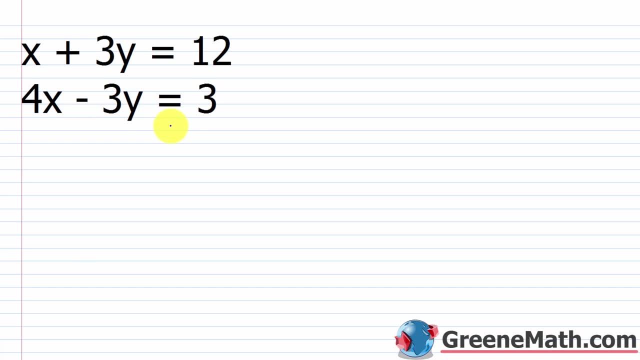 Are they perpendicular Or are they just nothing? So I would solve each for y Again, we're looking for y equals mx plus b. So for this one I have x plus 3y equals 12.. I subtract x away from each side. That'll cancel. I'll have 3y. 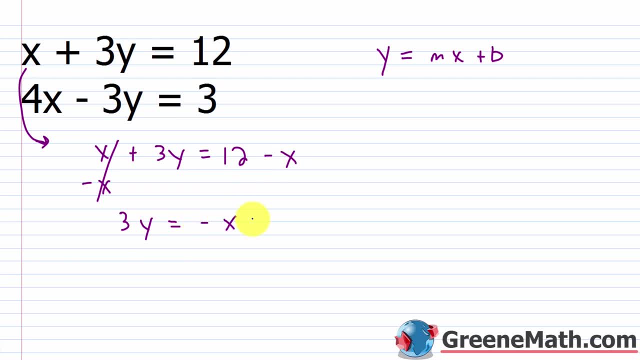 is equal to. Let's switch the order here. I'll put negative x plus 12. And then I'll divide each side by 3.. So this is going to cancel. I'll write y is equal to. I'm going to put a 1 there, So I. 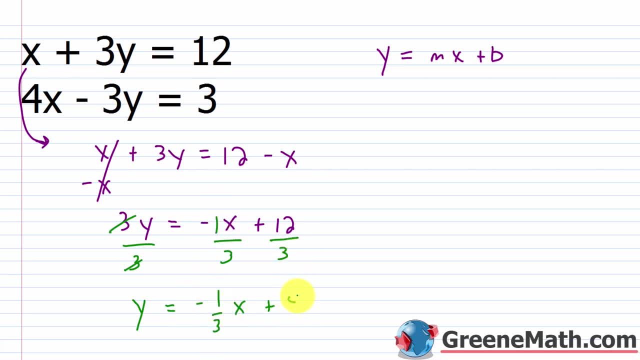 put negative 1 third x plus 12 over 3 is 4.. Let's go ahead and write this. Let's erase everything here. So again, y is equal to negative 1 third x plus 4.. All right for the next one. let's go ahead and do that over here. So 4x minus 3y is equal to 3.. 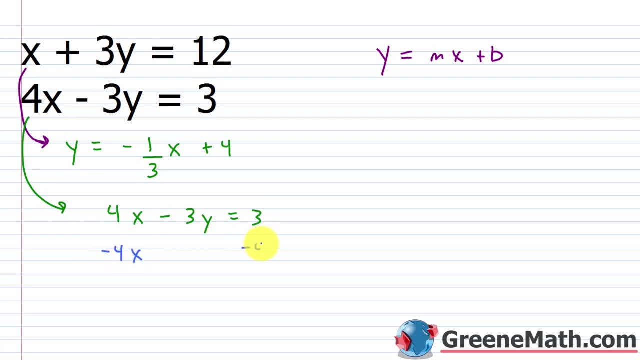 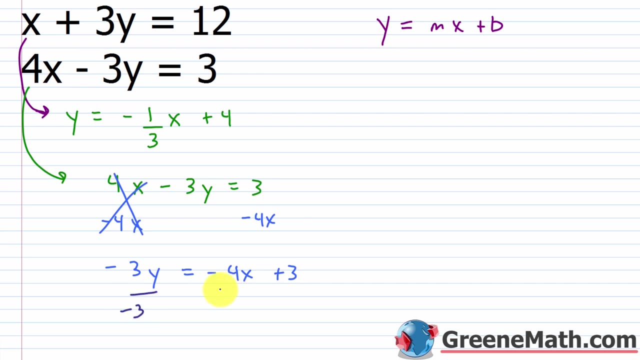 Let's subtract 4x away from each side. That's going to cancel. I'll have negative 3y is equal to negative 4x plus 3.. And what I want to do now is I want to divide both sides by negative 3.. 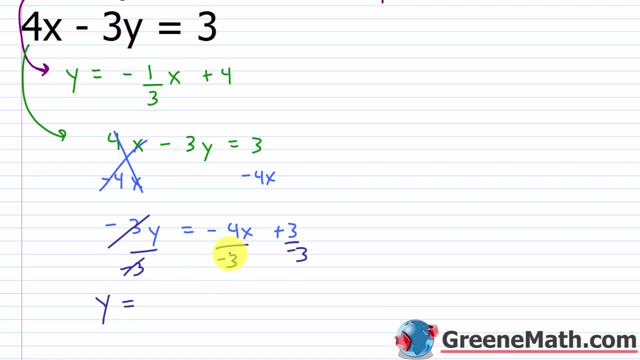 This will cancel. with this, I'll have: y is equal to negative, 4 over negative, 3 is 4, thirds and times x, And then 3 over negative, 3 is negative, 1. So minus 1.. Let's erase all this. 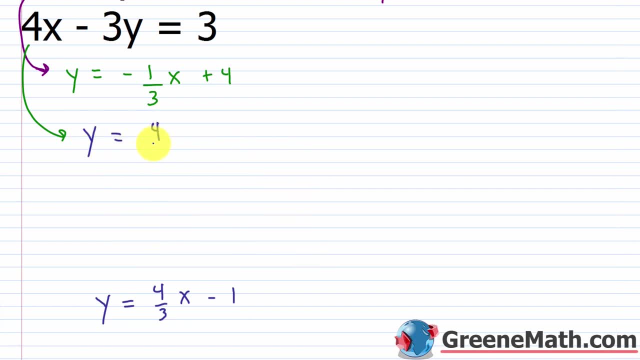 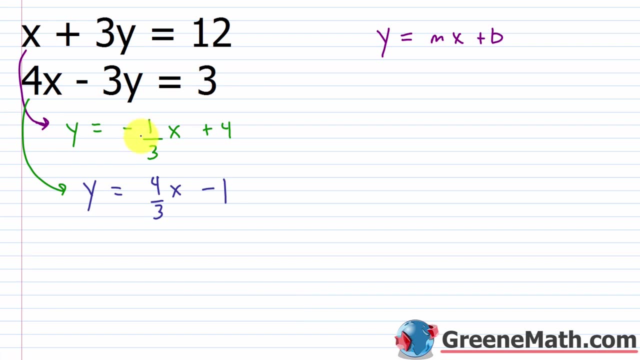 And let's write this here. So we have y equals 4 thirds, x minus 1.. So, looking at, let's do it again. So I want to do this over here. I want to divide both sides by negative 3. slopes, what can we say? We have negative 1 third and we have 4 thirds. So I know they're not the. 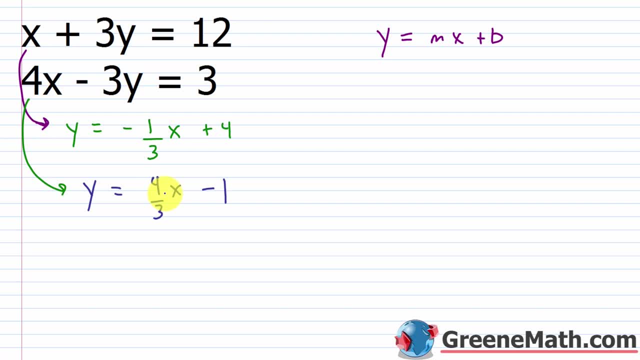 same, so they're not parallel lines. But would the product be negative 1?? So if I took negative 1 third, which is the slope from here, and I multiplied it by 4 thirds, which is the slope from here, would that be equal to negative 1?? Well, if I multiply here, negative 1 times 4. 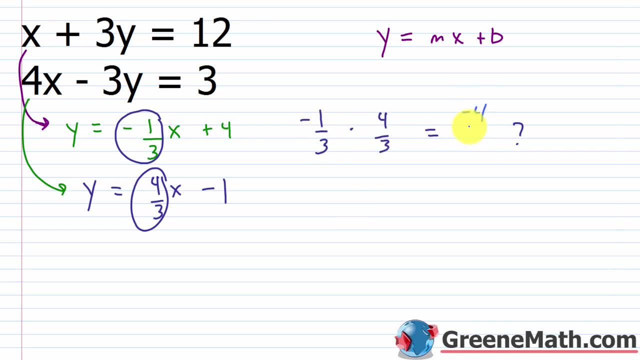 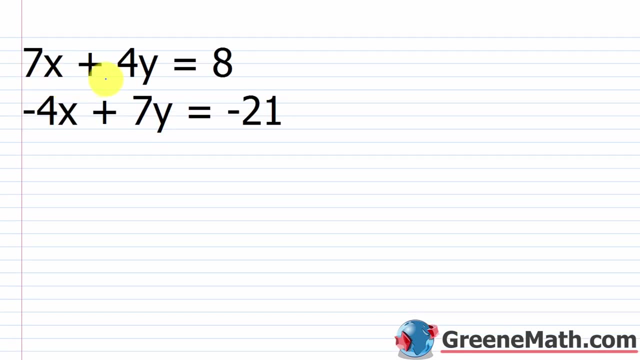 is negative 4.. 3 times 3 is 9.. So I end up with negative 4 ninths. So the answer to that is no, They're not parallel, They're not perpendicular, They're really neither. All right, let's take a look at one more. So we have 7x plus 4y equals 8, and we have negative. 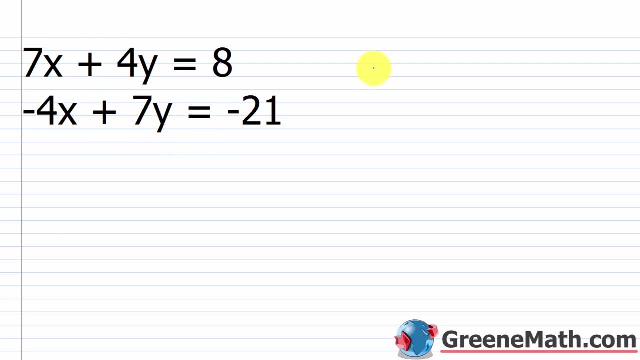 4x plus 7y equals negative 21.. So again I want to solve each for y. I want y equals mx plus b. So if I solve this I get negative. 4x plus 7y equals negative 21.. 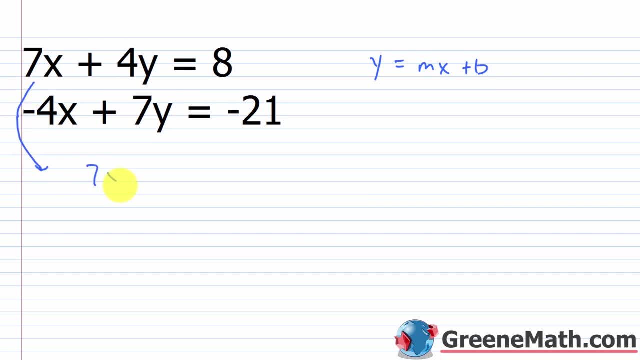 So if I solve this, I get negative 4x plus 7y equals negative 21.. So if I solve this, I get negative 4x plus 7y equals negative 21. So if I solve this guy for y, I would have again 7x plus 4y equals 8.. Let's move 7x. 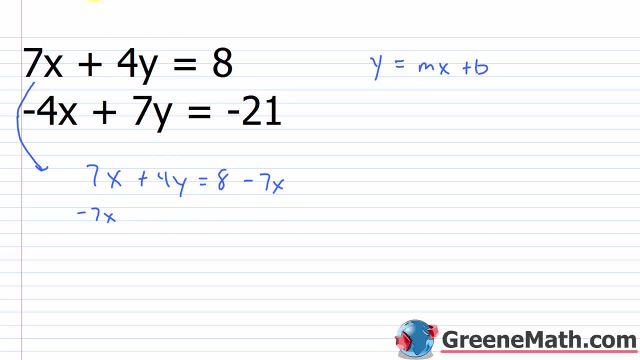 over to the other side. So I subtract away from each side. This will cancel. I will have. 4y is equal to negative 7x plus 8.. Then let me divide each side by 4.. So this will cancel. I'll have. 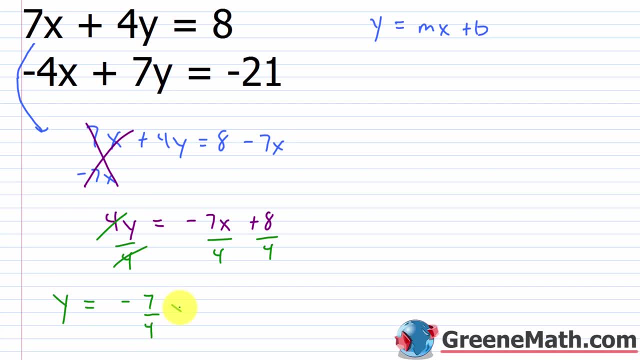 y is equal to negative 7, fourths times x plus 8 over 4 is 2.. Let's write what this is. Just drag this up here. All right, now. let's go ahead and do this one now. So I have negative. 4x plus 7y equals negative 21.. And again, let me add 4x to each side of the. 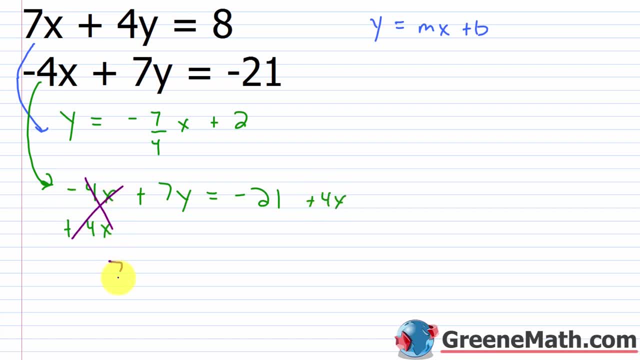 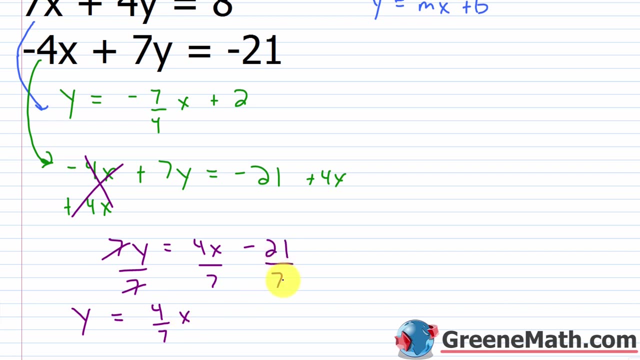 equation That's going to cancel, I'll have: 7y is equal to 4x minus 21.. I'll divide each side by 7.. That'll cancel. So with that I'll have: y is equal to 4 sevenths x negative 21 over 7 is negative 3.. 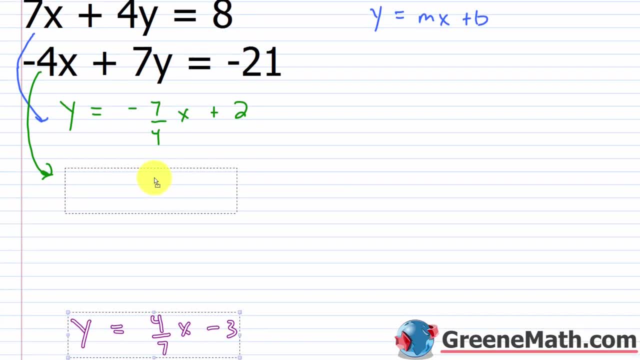 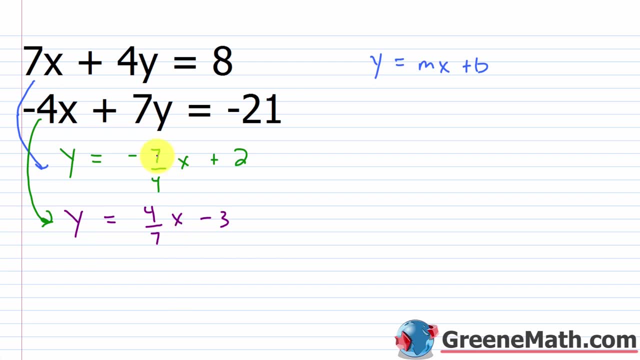 So let me erase this and I'll drag this up here. So y equals 4 sevenths x minus 3.. So let's look at the slope in each case. This one, it's negative 7 fourths. This one, it's 4 sevenths. 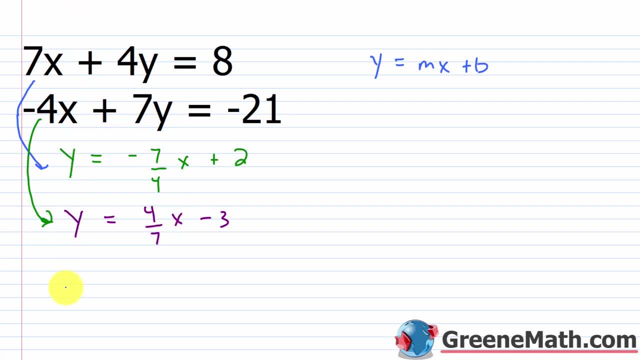 Most of you can see that if I multiply those two together, I'm going to get negative 1, right, If I take negative 7 fourths and I multiply it by 4 sevenths, this cancels with this. this cancels with this. I'm just left with a negative 1.. 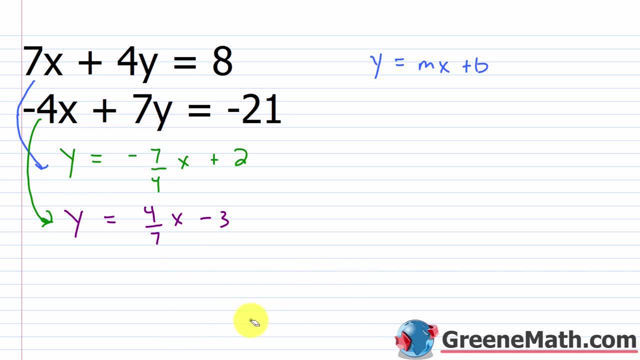 So, if the product of the slopes is negative 1,, we have something known as perpendicular lines. So perpendicular, And what this means is that these two lines will intersect at a 90 degree angle. Okay, For those of you who have never seen this or taken geometry before I'm going to graph, 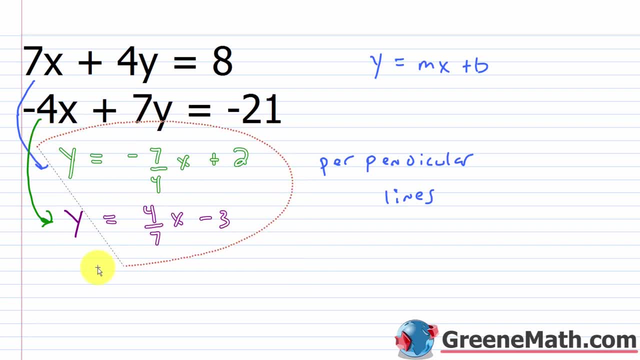 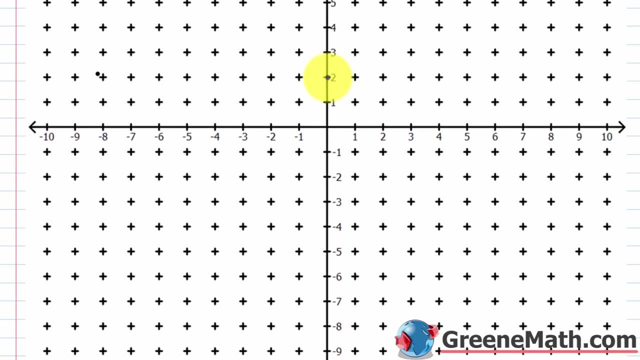 this real quick so that you can see it All right. So let's take these two down to the coordinate plane, All right? So for this one we have a y-intercept of 0 comma 2.. So that's going to be right here. 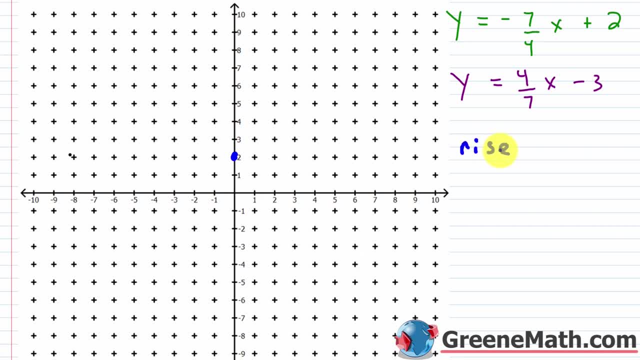 And then my slope. my rise over run is negative 7 fourths. So if I start here and I rise negative 7, I go down 7 units, So 1, 2.. 3,, 4,, 5,, 6, 7.. 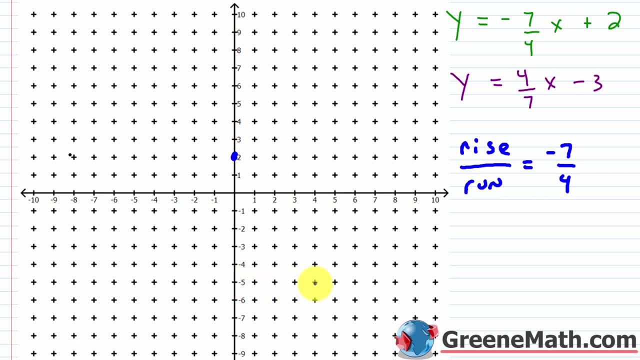 Then I run 4.. So I go to the right: 1,, 2,, 3,, 4.. So that's a point. Now I'd go off the coordinate plane that I have if I go down 7 and go to the right 4 again. 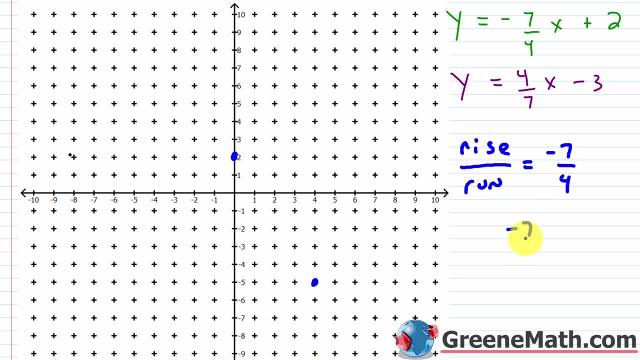 So what I'm going to do? again, I'm going to use a trick. If I have negative 7 over 4, that's equal to 7 over negative 4.. Okay, So I could start here and I could rise 7.. 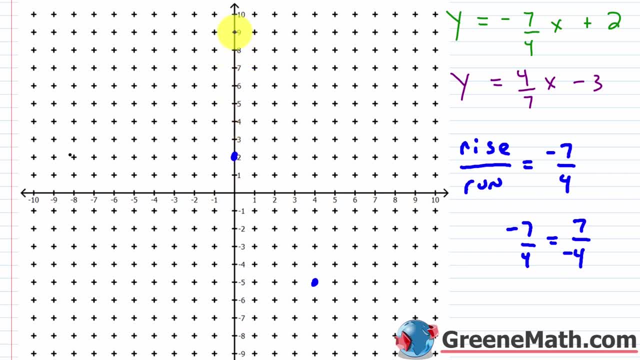 1,, 2,, 3,, 4,, 5,, 6,, 7.. And I could run Negative 4,, which means I go to the left 1,, 2,, 3,, 4.. So let me label this. 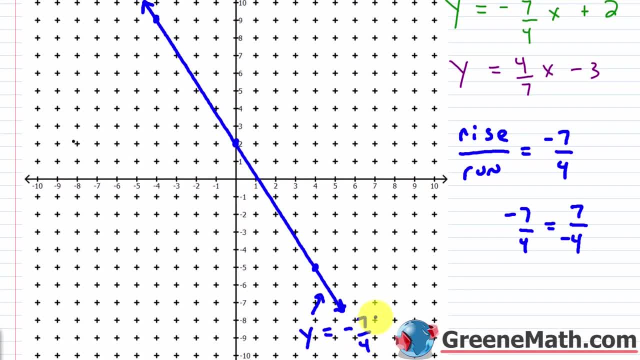 This is y is equal to negative 7 fourths x plus 2.. All right, So for the other one, let me kind of erase this part because it's going to change- We have a y-intercept that occurs at 0 comma, negative 3.. 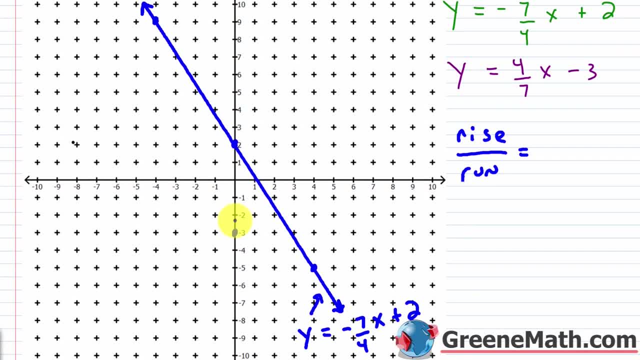 So that is going to be right here. And then the next part is: The slope is now 4 sevenths. So let me change colors For 4 sevenths. I'm going to rise 4.. So rise 1,, 2,, 3,, 4.. 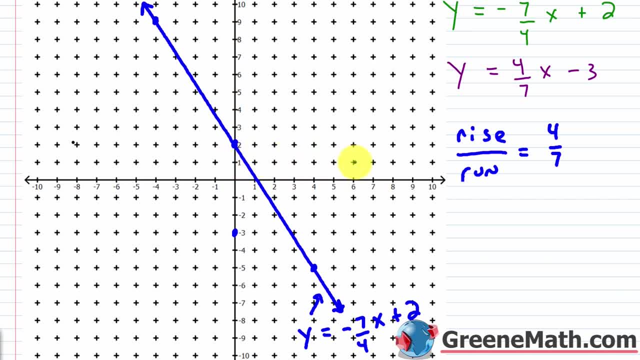 Go to the right: 7.. 1,, 2,, 3,, 4,, 5,, 6,, 7.. It's right there. And again I can reverse that. I can put: 4: sevenths is equal to negative 4 over negative 7.. 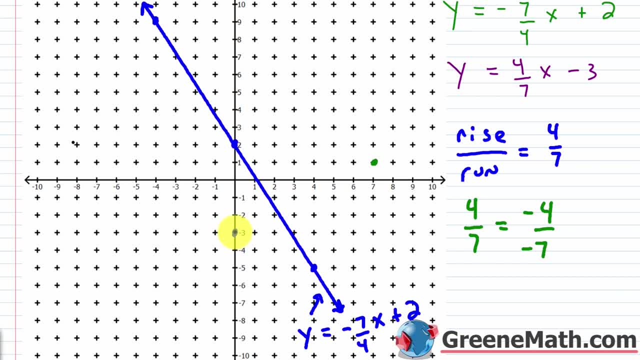 Negative over negative is positive. So I could start here and I could go down, 4.. Down 1. 1,, 2,, 3,, 4.. And I could go to the left, 7.. 1,, 2,, 3,, 4,, 5,, 6,, 7.. 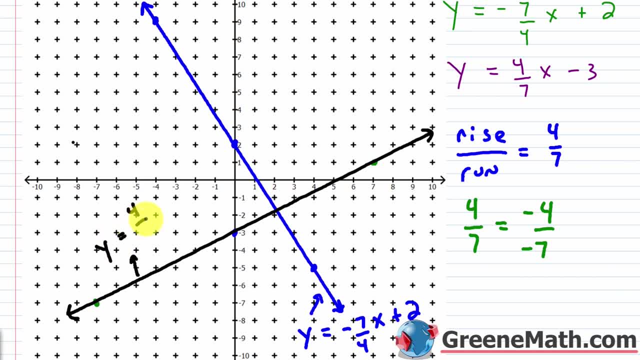 Again, this is going to be: y is equal to 4 sevenths x minus 3.. Now I want you to look at something real quick Again, if you've never seen a 90-degree angle, or right angle as it's called- 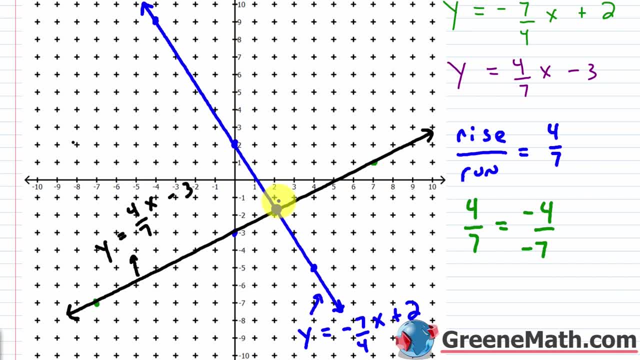 you want to look at the point of intersection Here, which is right there, It forms a 90-degree angle, which is displayed with this symbol here. This is a 90-degree angle, And if there's one 90-degree angle, it's such that it's a 90-degree angle at all of them. 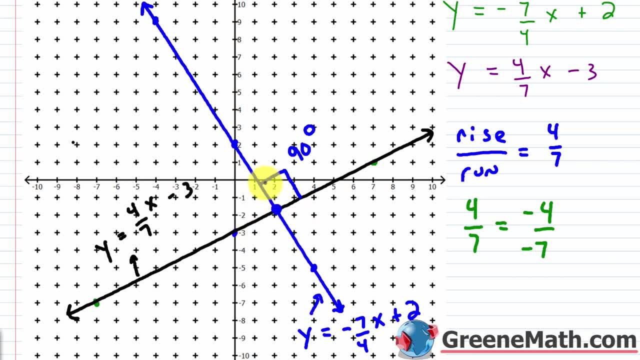 So this is a 90-degree angle. This is a 90-degree angle And this is a 90-degree angle, And you'll talk more about that in your geometry class. I mean, we really don't go way into this in algebra, but it's something you need to know to kind. 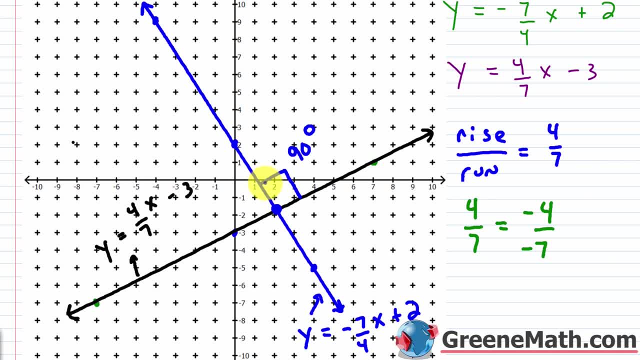 of understand what perpendicular is, What perpendicular lines are. It's again such that at the point of intersection, which is right here, you're going to form a 90-degree angle And in fact you're going to form four of them. 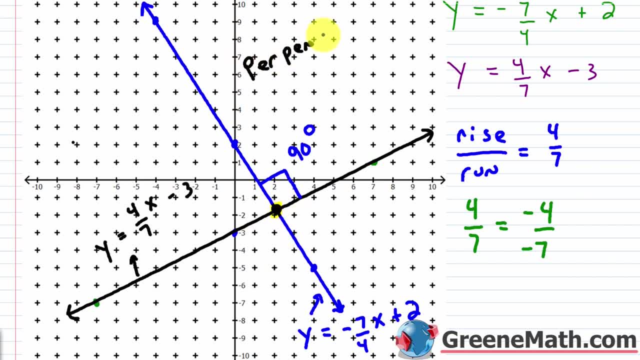 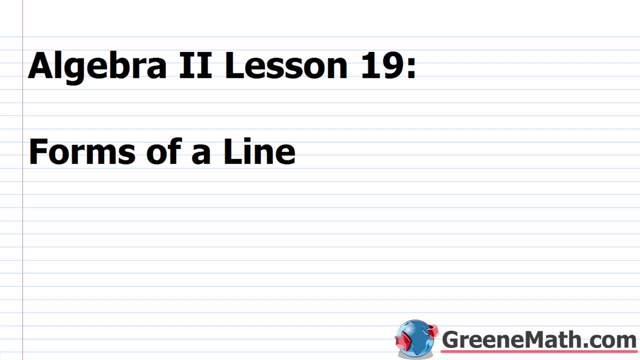 So these are perpendicular lines. Hello and welcome to Algebra 2, Lesson 19.. In this video, we're going to learn about forms of a line. So we talked about this already in Algebra 1, and we're going to revisit for Algebra. 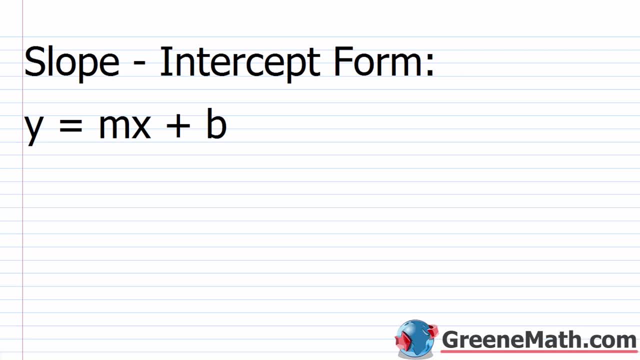 2. When you talk about a linear equation in two variables, there are ways you can algebraically manipulate this equation and put it in different forms. So we have slope-intercept form, We have point-slope form And then we have standard form that we're going to talk about today. 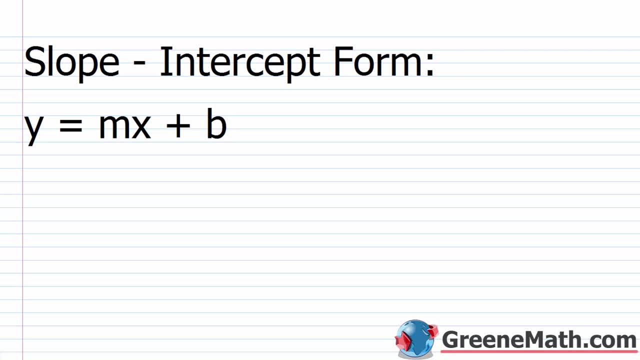 So, based on what form it's in, you can use it for certain things, get different information from it And when we start out with slope-intercept form, we know the slope and we know the y-intercept, And we've already talked about this form in the previous two lessons. 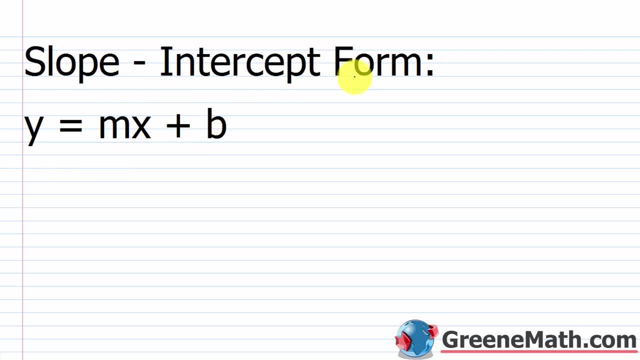 So we have: y equals mx plus b. Again, this is slope-intercept form. So when I have something like this, I know the slope which is denoted as m- This is given as the coefficient of x- And I know the y-intercept is going to occur at. 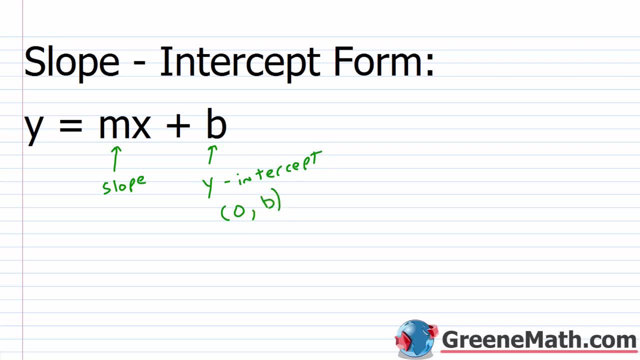 How do I know that? Well, if I want to find the y-intercept again, I have y equals mx plus b. To find the y-intercept, I just plug a 0 in for x. 0 times. anything is 0.. 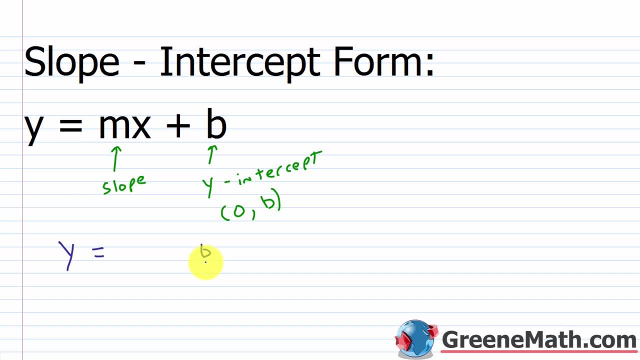 So this would go away. Then I'd have y equals b. So that's why I know that the y-intercept occurs at. So, as an example, if I had y equals 3x plus 2, I know that the slope is 3 and the y-intercept 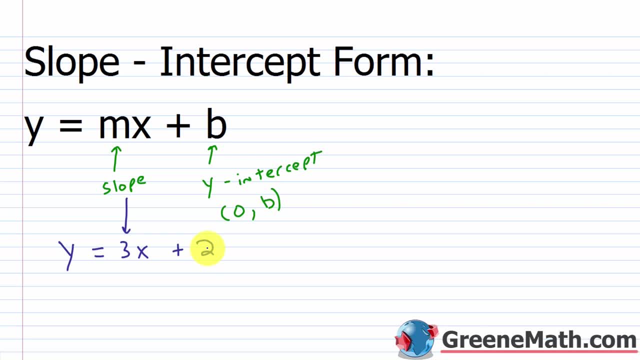 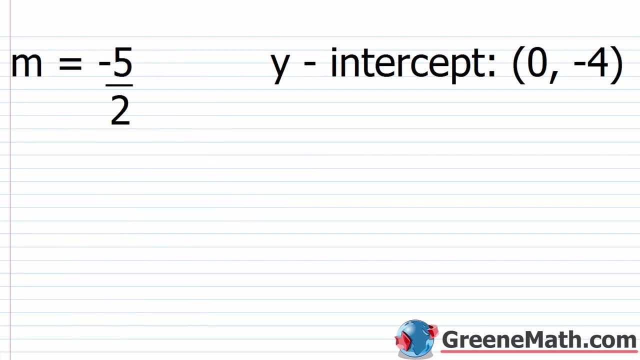 occurs at. Very, very simple. If I have something like y-intercept, y equals 1 fifth x minus 7.. The slope is 1 fifth. The y-intercept occurs at Super, super easy. So let's say we wanted to take this information and write an equation in slope-intercept form. 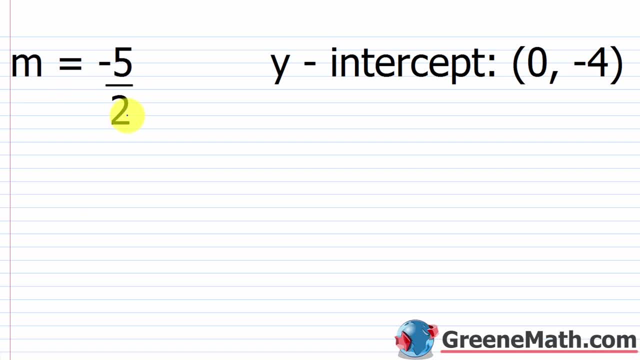 So we have m, which is the slope is equal to negative 5 halves. We have a y-intercept, that's So just match this up. We have again: y equals mx plus b, And do it like this when you first start, so you don't forget. 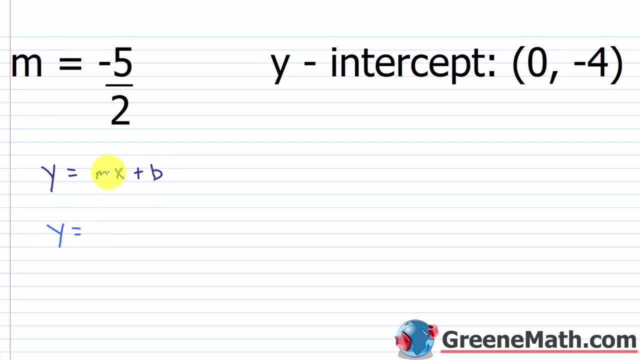 So you have that in your head and you say, OK, well, y equals. I know m is slope, So m is equal to negative 5 halves. So I'm going to put negative 5 halves here, then times x, Then I have plus b. 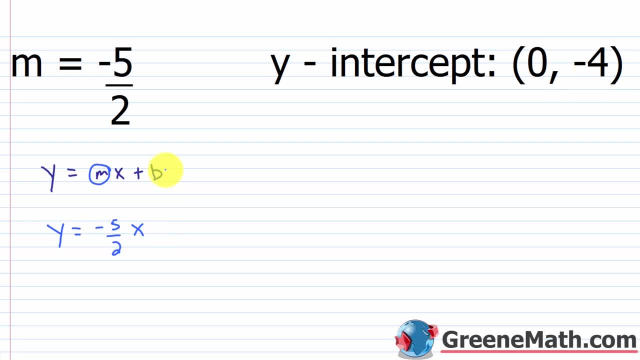 The y-intercept occurs at. So b is really the y-coordinate there, so just negative 4.. So I'm going to put for plus b, I'm going to put minus 4.. So using this information, I write: y equals negative, 5 halves x minus 4, because negative. 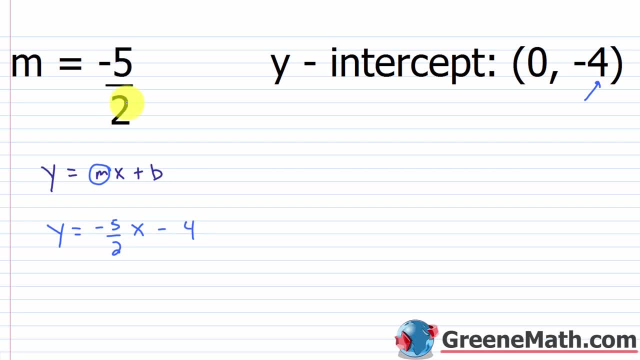 5 halves is the slope, which is m, and the y-intercept occurs at 0 comma negative 4.. All right, let's take a look at another one. We have a slope m that is equal to negative 4 thirds and we have a y-intercept that occurs. 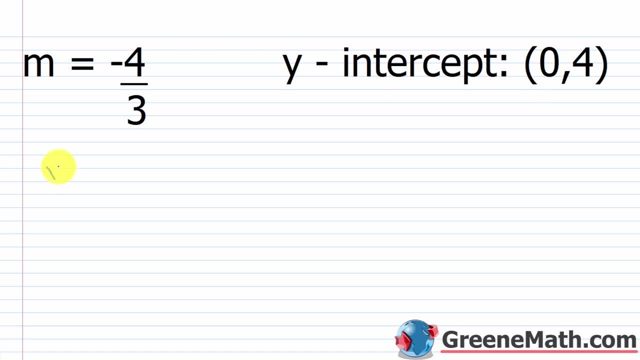 at 0 comma 4.. So again, let's match this up. We have y equals mx plus b, So this would be y equals. for m, I have negative 4 thirds times x, And then for b I have 4, so plus 4.. 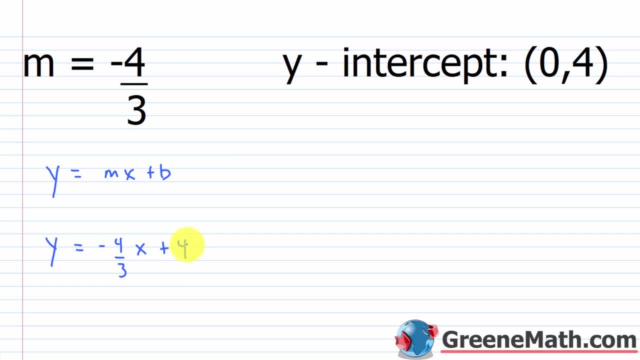 So y equals negative 4.. So y equals negative 4 thirds x plus 4.. All right, what about this one? We have m equal to 1, and we have a y-intercept at 0 comma 3.. So again, if I have y equals mx plus b, m is 1 now. 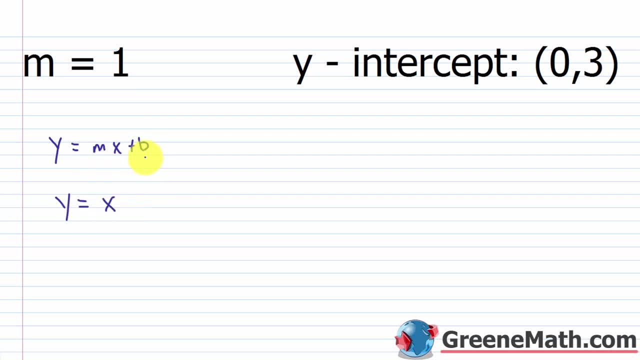 So y equals 1x is just x, and then plus b, b is 3 here, so plus 3.. So y just equals x plus 3.. So again, slope-intercept form is super easy. So you know, if you take a linear equation of two variables and you solve it for y. 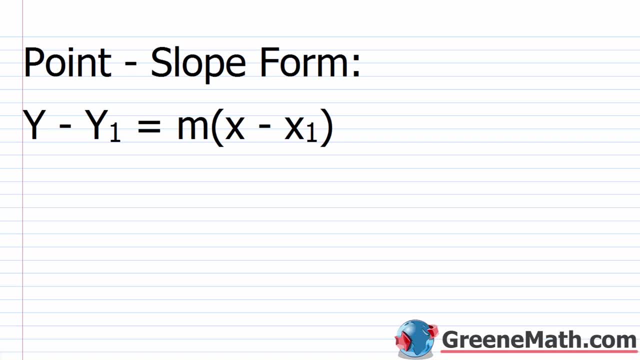 you get slope-intercept form y equals mx plus b. It makes it easy for you to know the slope, the y-intercept. It also makes it easy for you to graph right. You have a point and you have the slope, so it's super easy to do that as well. 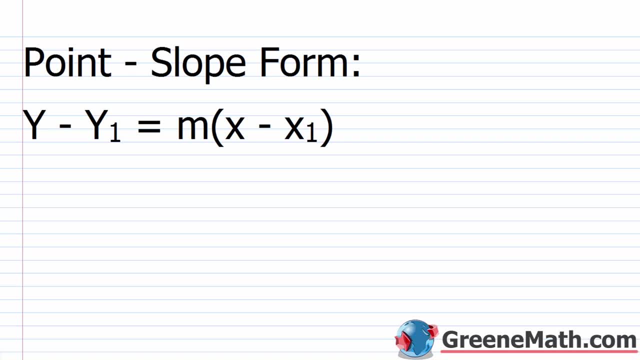 So now I want to talk about kind of the next form of a line, which is point-slope form. So you're going to use this in two specific scenarios: One, you know the slope and one point on the line. The other is you have two points. 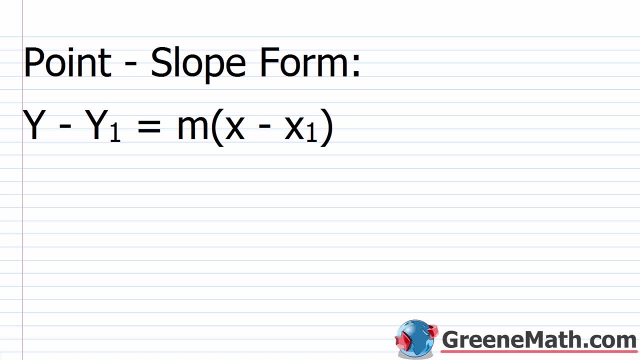 You're not going to go straight into slope-intercept form if you don't have all the right information. So with point-slope form I plug in for y sub 1, x sub 1, and m, and then I can solve. 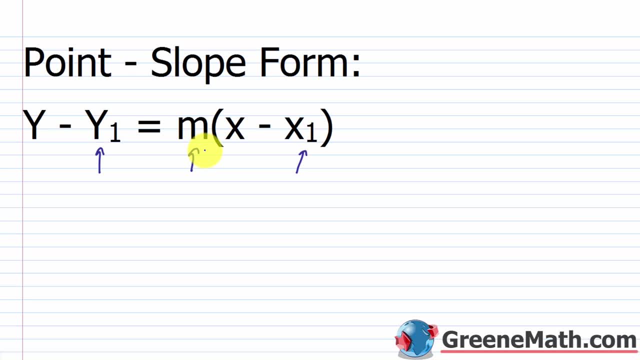 for y and I can get slope-intercept form. So we have: y minus y sub 1 equals m times the quantity x minus x sub 1.. So let's go down here. So let's say we have a slope m, that's 1 half. 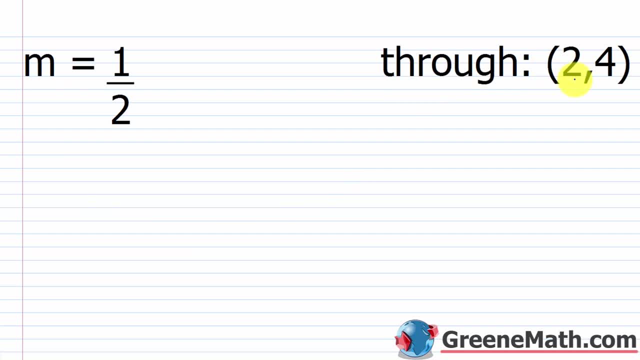 So let's go down here. So let's say we have a slope m, that's 1 half, And this line goes through the point 2, comma 4.. So what we want to do here again, just copy it to start. 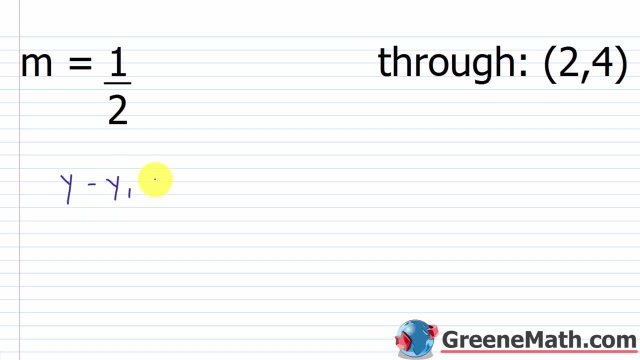 So point-slope form is: y minus y sub 1 is equal to m times the quantity x minus x sub 1.. So the y sub 1 and the x sub 1 come from the point that you're given. So you kind of think about 2 comma 4.. 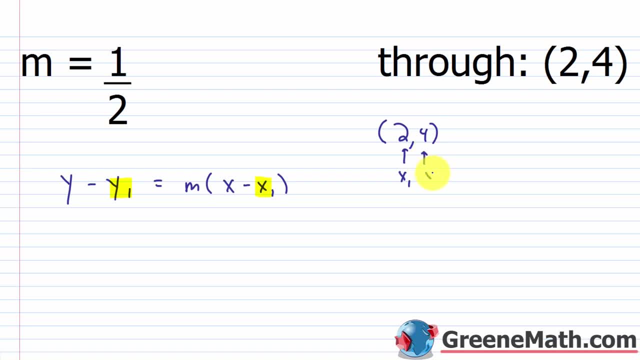 This is a point on that line. So this is your x sub 1.. This is your y sub 1.. And this is your m. So all that stuff is just going to get plugged in, So let me highlight m as well. 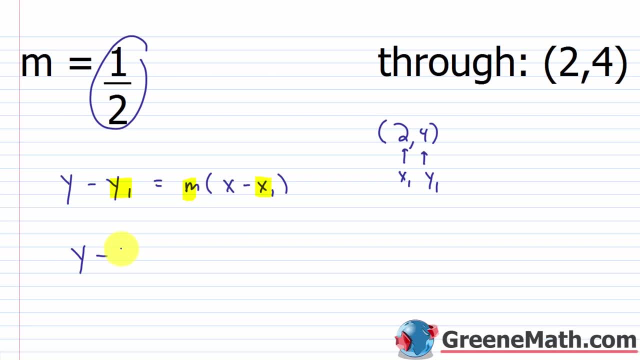 So I'm going to have y minus y sub 1.. For y sub 1, I'm plugging in a 4. And this equals: for m, I've got 1 half times the quantity x minus. for x sub 1, I'm plugging. 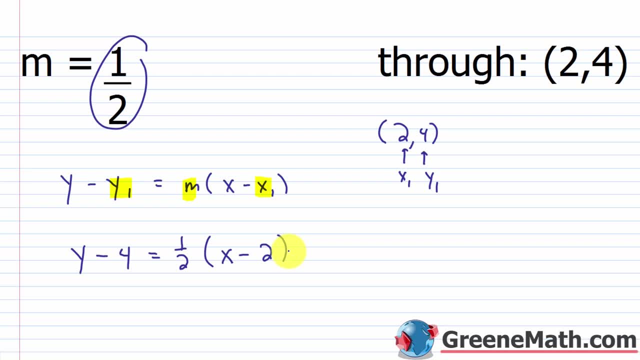 in a 2.. Now, if your teacher asks you for point-slope form, stop, here, You've arrived. This is point-slope form. so if you're asked for that specifically, you're done okay, but in most cases they want you to solve. 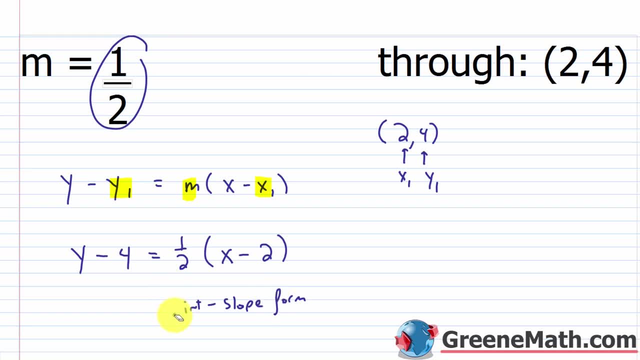 for y and put it in slope intercept form. this is a scenario where you did not know what the y intercept was. you're just given a point in the slope. okay, so you've got to go through it this way. so now what i'll do is i'll have: y minus four is equal to one half times x is one half x. 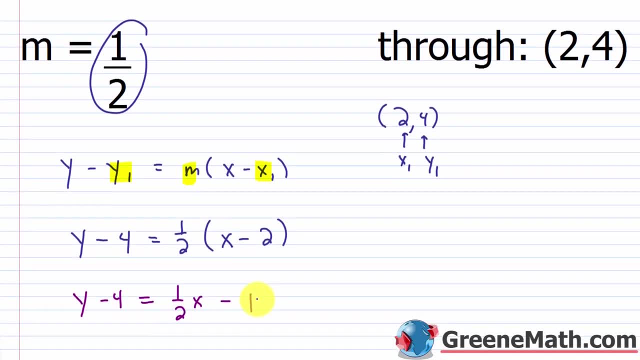 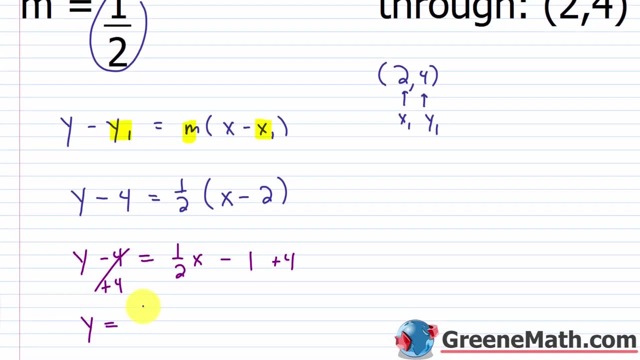 minus one half times two is just one. so i add four to each side of the equation, that'll cancel and i'll have: y is equal to one half x. negative one plus four is going to give me three. so plus three. so now it's in slope intercept form and i can also add that the y intercept occurs at zero. 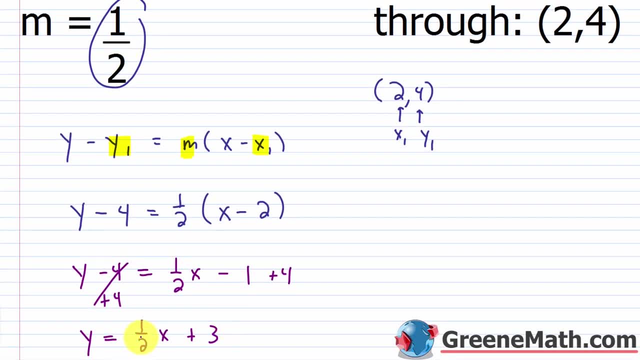 three. so i know the slope which is one half. it matches up there. i know a point on the line is two comma four and you could check that. plug in a two here. two times a half is one, one plus three is four. so that works out. and i also know the y intercept would occur at zero comma three. so again, y equals one half x. 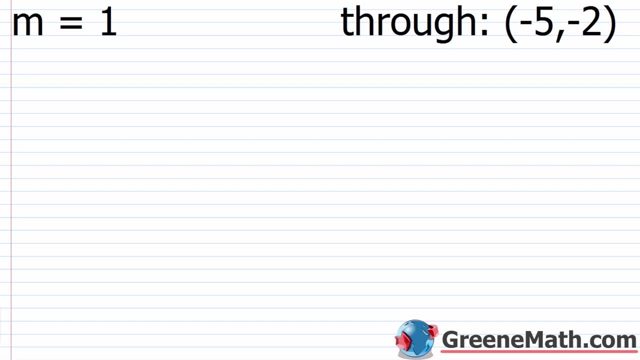 plus three. all right, let's take a look at another. so suppose i had a slope m, that's one. and this line goes through the point negative five, comma, negative two. so again, i'm going to label this x sub one, y sub one and i'm going to plug into the point slope form. so that's going to. 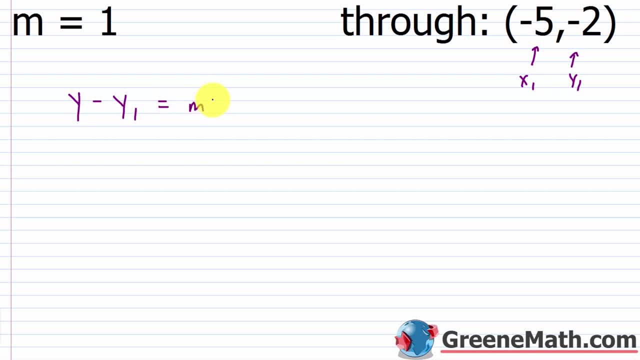 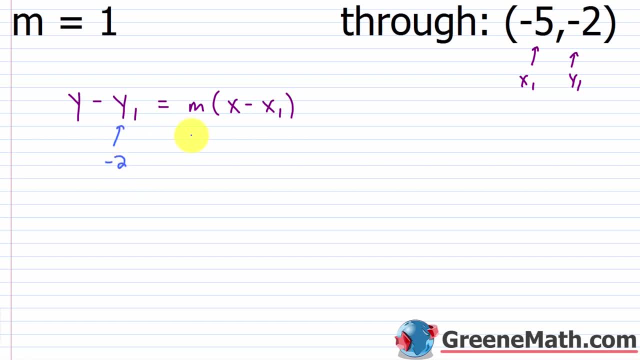 i'll give you the y i'ts of one x minus x plus y minus x plus y minus y plus. then y minus y minus y plus m. no one should be past minus one n, And I guess what I should say in these cases is that 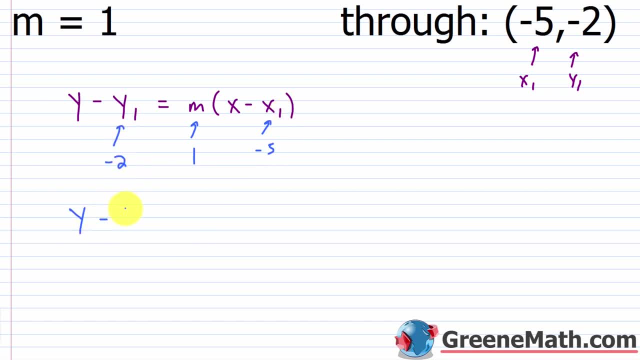 each graph might be 1 minus x plus one, x minus y minus x is getting leaving out of SPEAKER, перем가지고 in ref grund, and so on for each graph. I'm going to focus a lot of my efforts on this. one, because here we go: one plus two is equal to three times x plus one y sub one peg Hiç. 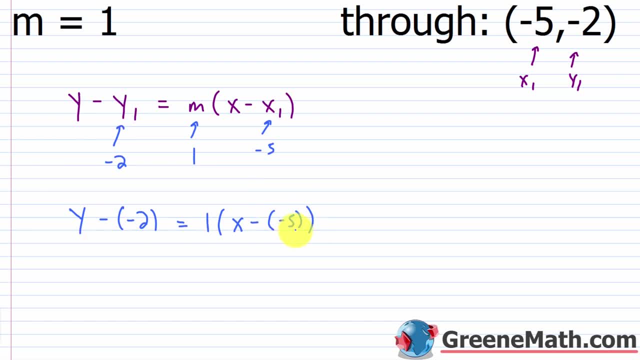 So again, this is point-slope form. If you're asked for that, you can stop. In most cases, you're asked for slope-intercept form, so keep going. So what I want to do is simplify. So this is: y plus 2 is equal to. 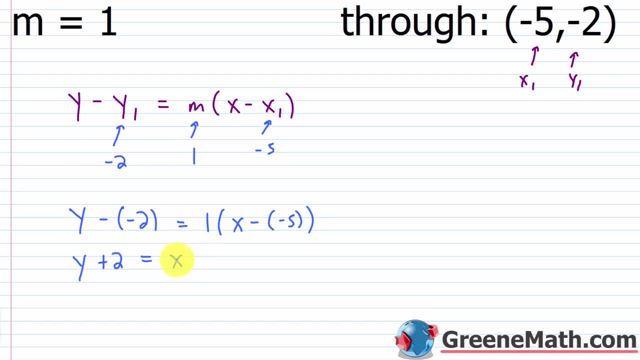 I can get rid of the 1, really, because 1 times anything is itself. So just x minus the negative 5 is plus 5.. So I just subtract 2 away from each side of the equation and I get y is equal to x plus 3.. 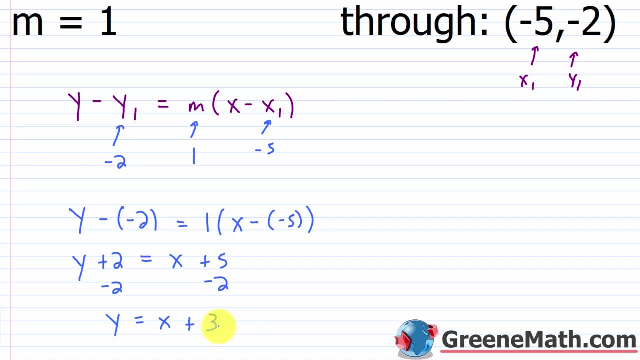 So now I know that the y-intercept occurs at 0,3.. We already knew the slope was 1, and we have a point on the line of negative 5 comma, negative 2, right. So if I plugged in a negative 5 there, negative 5 plus 3 is in fact negative 2.. 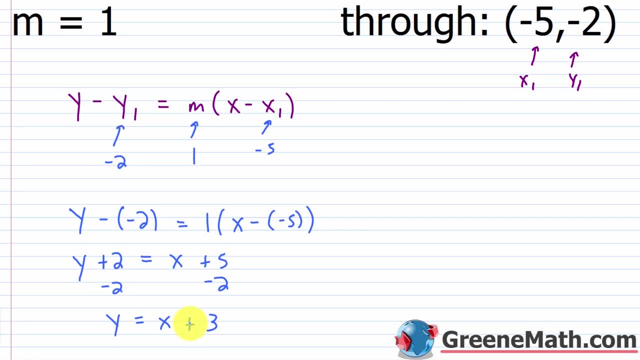 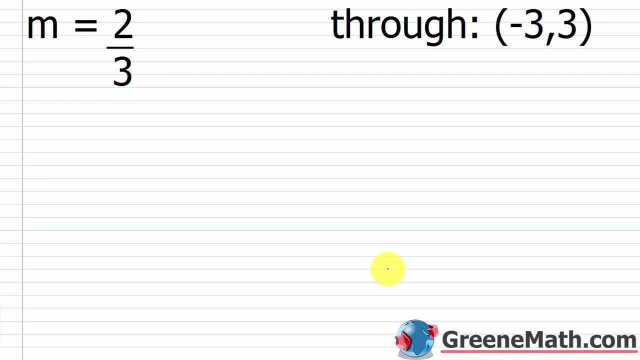 So again, the equation of this line in slope-intercept form is: y equals x plus 3.. Let's take a look at another one. So we have m equals 2 thirds and it passes through the point negative 3 comma 3.. 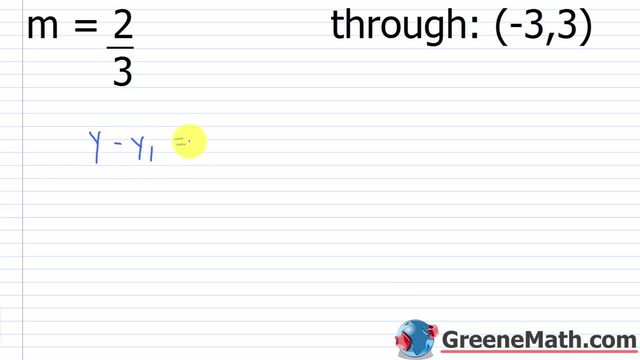 So again we have: y minus y sub 1 is equal to m times the quantity x minus x sub 1, and I'm going to label this. This is x sub 1, y sub 1, and I'm just going to plug in. 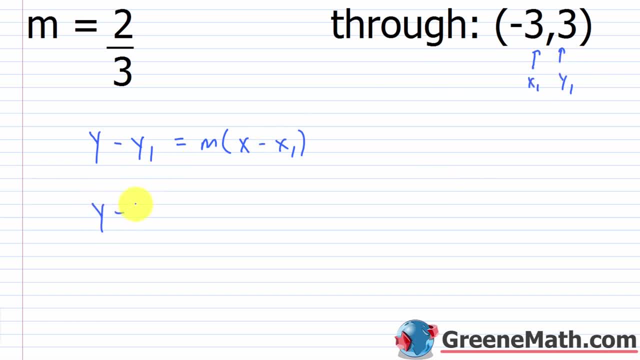 So I'll have y minus for y sub 1, I have 3, is equal to m, which is 2 thirds times the quantity x minus for x sub 1, I have a negative 3.. So minus a negative 3.. 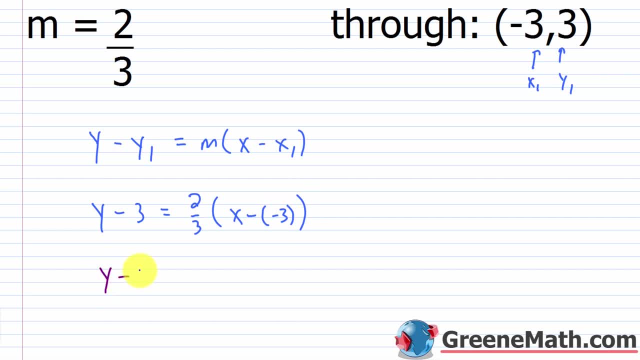 All right. so now we have: y minus 3 is equal to 2 thirds times x, is 2 thirds x, and then we'll have 2 thirds times 3.. Right, minus a negative 3 is plus 3.. So if I had 2 thirds times 3, the 3's would cancel and be left with 2, so plus 2.. 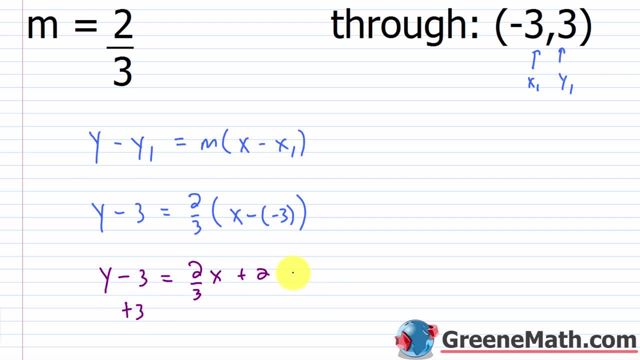 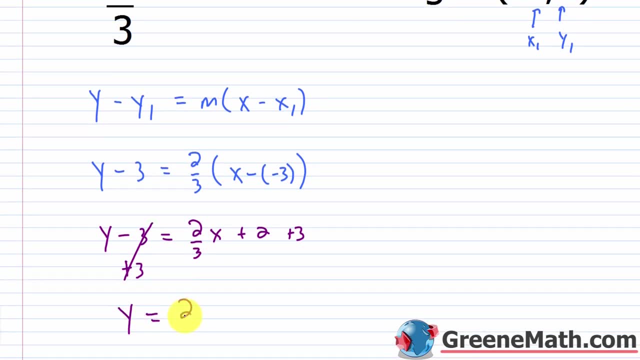 All right, so now all I need to do is just add 3 to each side. that'll cancel, and I'll end up with: y is equal to 2 thirds x 2 plus 3 is 5, so plus 5.. 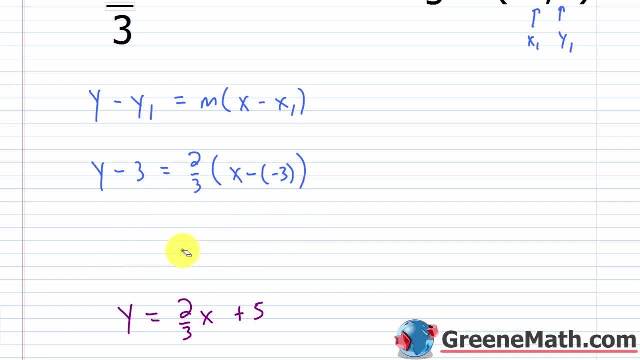 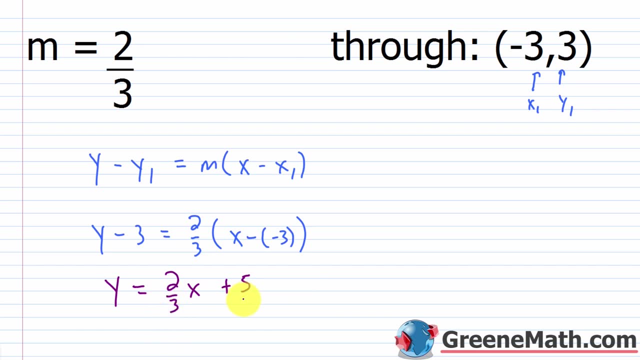 So what can we say here? We kind of erase this so I can fit everything on the screen. Scroll down, Hold this up. Well, we can say that the slope is 2 thirds. the y intercept occurs at 0, 5,. 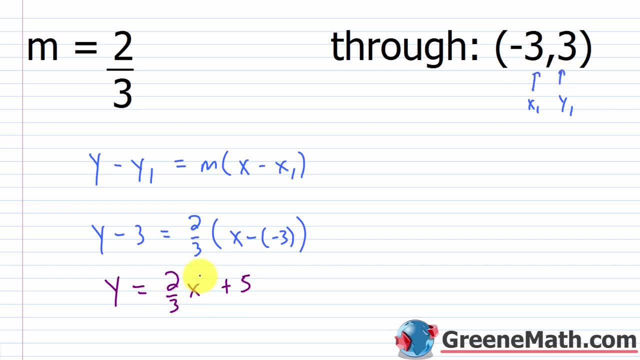 and we have a point negative 3,, 3.. So if I plugged in a negative 3 there, negative 3 times 2, thirds would be negative 2, negative 2 plus 5 would be 3, so that does work out. 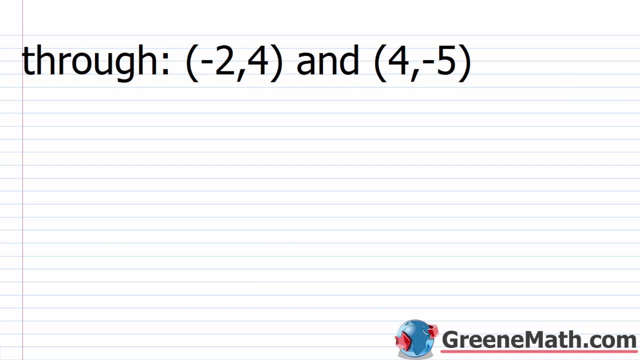 All right. so here's another scenario. you're going to be given It's kind of a curveball they'll throw at you. Let's say you're just given two points, So you have through the point negative 2, 4, and 4, negative 5.. So the first thing you're going to do is you're going to do a curveball. So the first thing you're going to do is you're going to do a curveball. So the first thing you've got to do is you've got to get a slope. 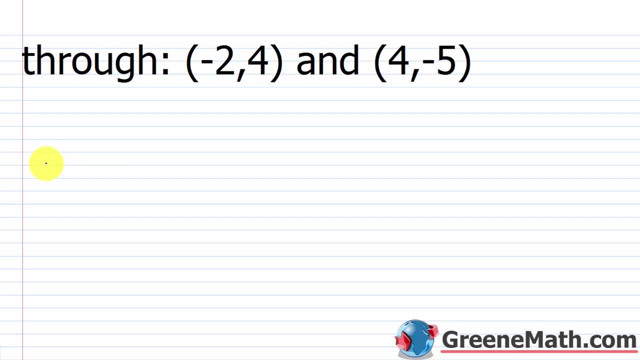 because you can't make it with this formula. You have: y minus y sub 1 equals m times the quantity x minus x sub 1.. So you're not going to make it. You've got to find out what m is. So to do that, we just use our slope formula. 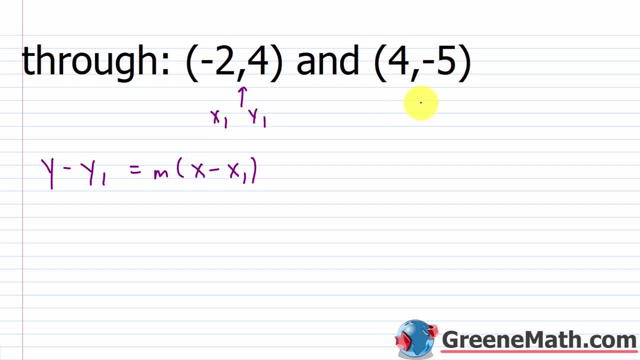 So I label one of these points as x sub 1, y sub 1, the other as x sub 2, y sub 2.. Now here's where it gets confusing. The way I label this here is- I'm going to use the slope formula. 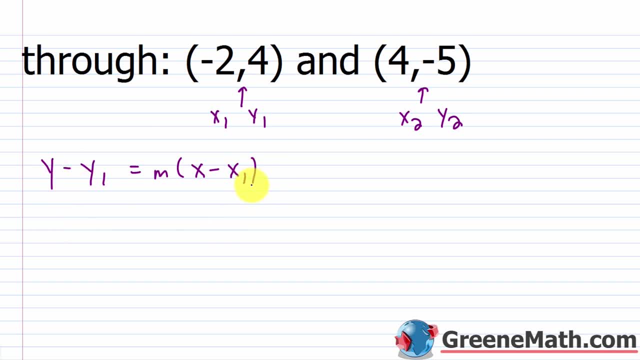 The way I label this here is: I'm going to use the slope formula. The way I label this here is: I'm going to use the slope formula. The way I label this here has nothing to do with my inputs over here. okay, I can label this: x sub 1, y sub 1, this: x sub 2, y sub 2.. 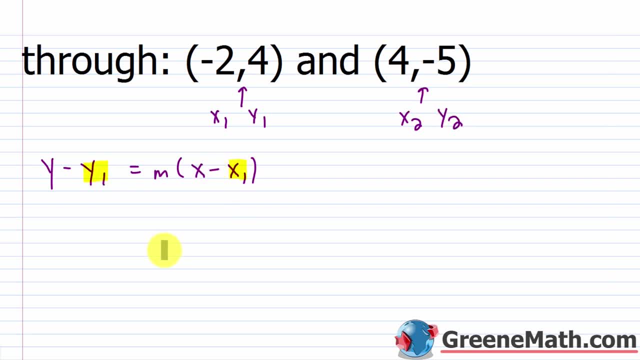 When I go to plug in for x sub 1, y sub 1,, it doesn't matter if I use this point or this point, It's irrelevant. So, knowing that, let's do the first step and just find out. So m is equal to remember the formula. 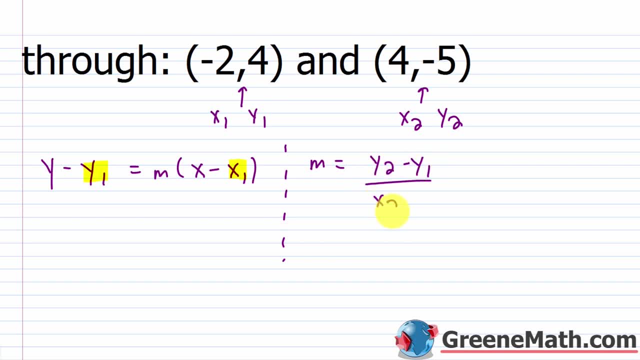 it's y sub 2 minus y sub 1, over x sub 2 minus x sub 1.. So m will be equal to y sub 2, is negative 5 minus y sub 1,, which is 4, over x sub 2,, which is 4, minus x sub 1,, which is negative 2.. 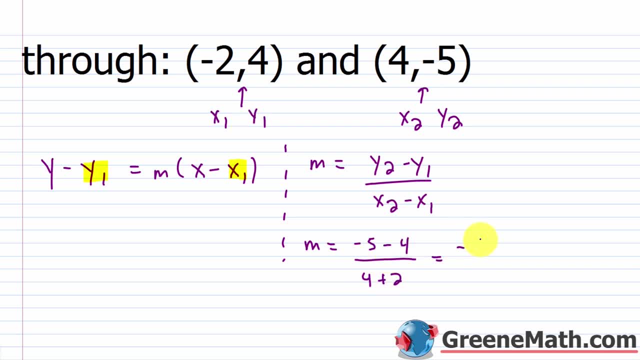 Minus the negative 2 is plus 2.. Negative 5 minus 4 is negative. 9 over 4 plus 2,, which is 6.. So each is divisible by 3.. Negative 9 divided by 3 is negative 3.. 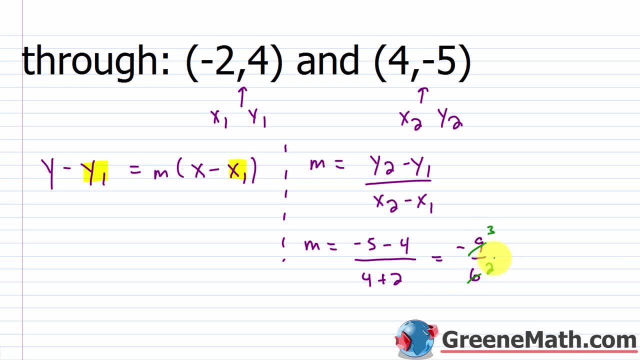 6 divided by 3 is 2.. So this is negative 3 halves for the slope. Let me erase everything And we can put that in: m equals negative 3 halves. Now, because we have this information now, we can plug in here: 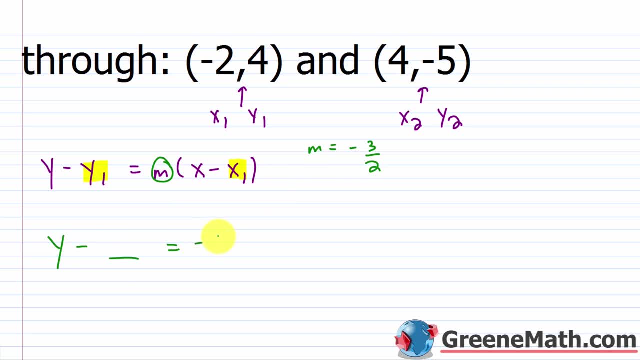 So y minus something equals negative, 3, halves times the quantity x minus something right for x sub 1.. Now I can plug in this point as x sub 1, y sub 1, or this point as x sub 1, y sub 1.. 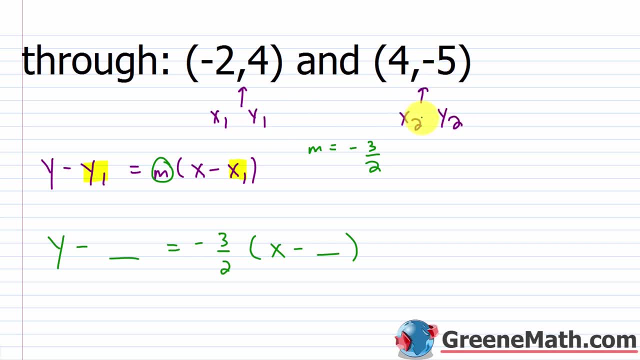 It does not matter that I labeled them this way, It's just a way to get the slope. It's irrelevant now. You can kind of choose a point and then forget the other. Either point would work. I can't stress that enough, because students really get stressed out over this stuff. 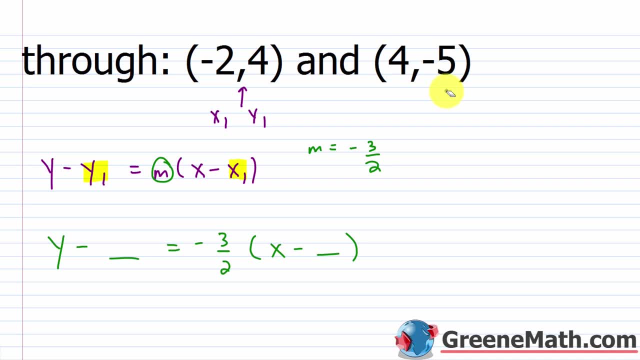 They're like: well, which one do I plug in? now What do I do? Just pick a point, plug it in. It'll look different in the point-slope form, but if you go into slope-intercept form it's going to be the same. 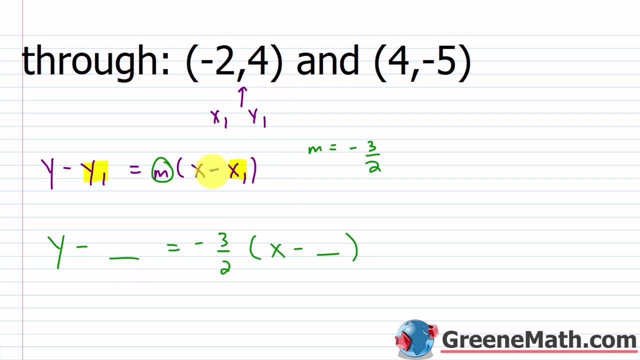 And I'm going to prove that to you right now. So let's start with this one. So let's say we have a 4 here, That's a y sub 1 we're plugging in. Let's say we have minus a negative 2 right here. 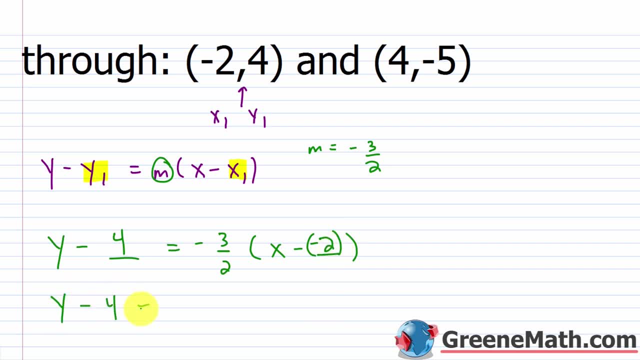 So doing that, I have y minus 4 is equal to negative 3 halves times x. And then this is plus. Let me write this as plus 2.. And then negative 3 halves times 2 would be minus 3, right. 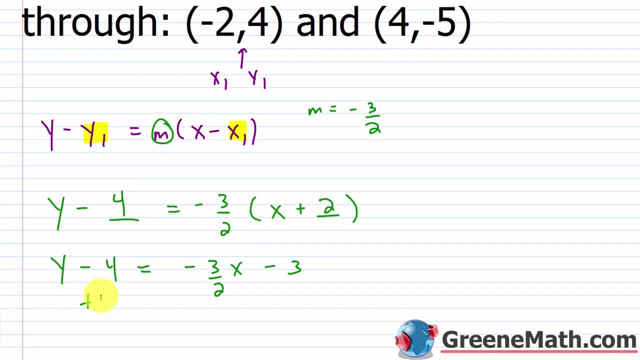 because the 2s would cancel. All right. so if I just add 4 to each side of the equation I'm going to end up with, y is equal to negative. 3 halves x. negative 3 plus 4 is plus 1.. 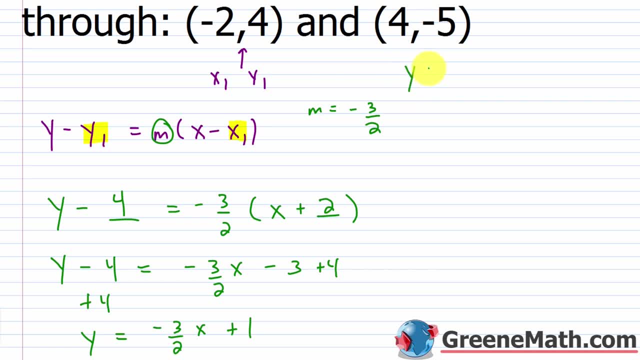 Now let's say I put this over to the side, So y equals negative 3 halves x plus 1.. And let's forget about this point. Let's just forget that it exists. Let's erase all this, and I'm going to show you that it doesn't matter if I choose this point. 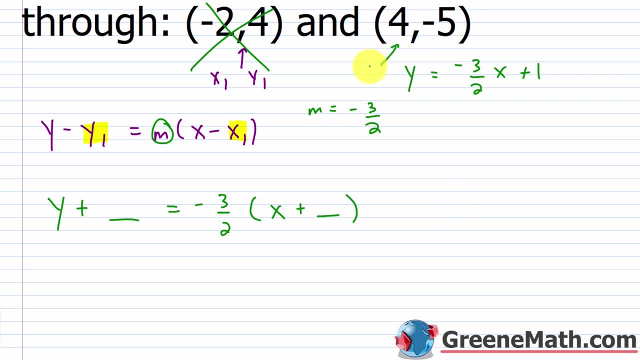 So now I'm going to choose this as x sub 1, y sub 1.. And remember, this formula is 1.. This is y minus y sub 1 equals m. We already know that's negative 3 halves times the quantity x minus x sub 1.. 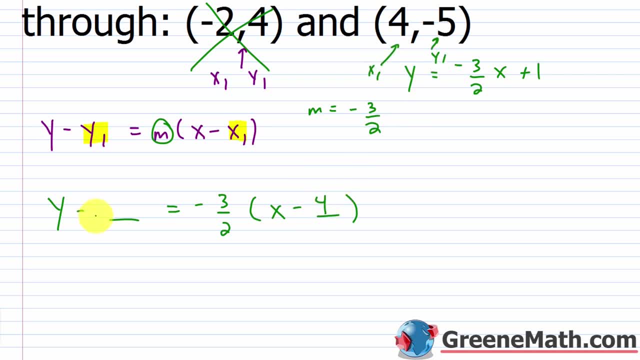 So x sub 1 is 4.. y sub 1 is negative 5.. So minus a negative 5 is plus 5.. So we'd have: y plus 5 is equal to negative 3 halves times x is negative 3 halves x. 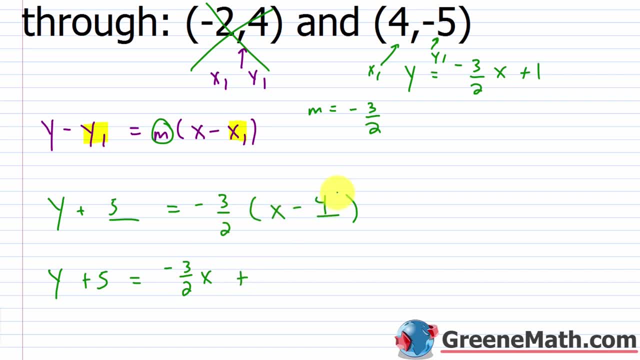 Then negative 3, halves times negative 4, we know that's positive. The 4 would cancel with the 2 and give me 2.. 2 times 3 is 6.. So as a last step here, let's just subtract 5 away from each side. 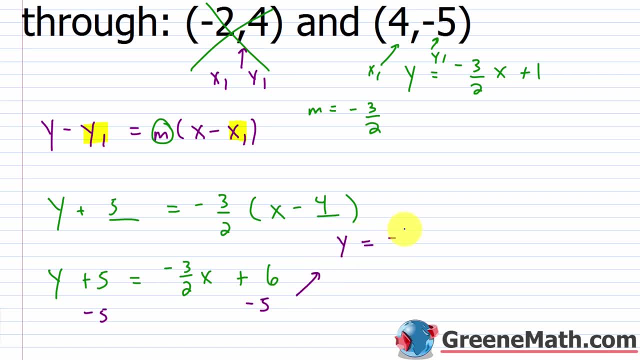 And that's going to give me that y is equal to negative. 3 halves x plus 6 minus 5 is 1.. Same thing here. Notice that it didn't matter which point I plugged in, for In point slope form it looks different because the inputs are different. 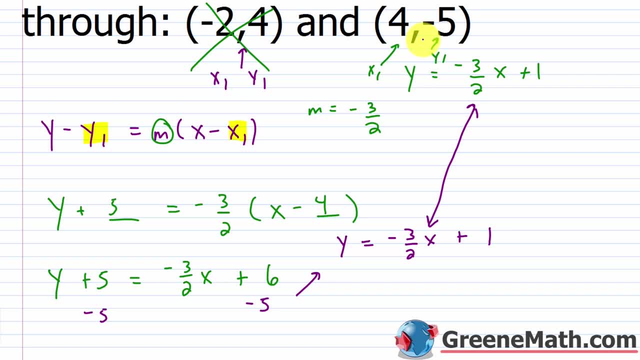 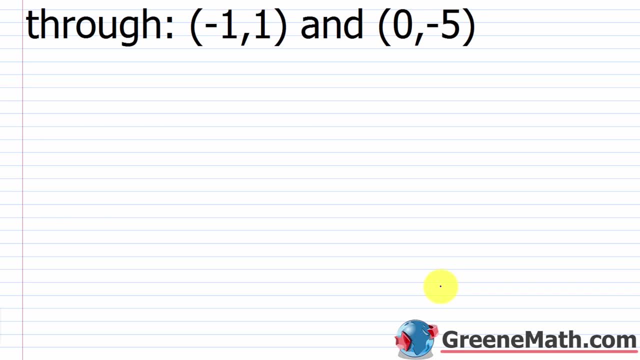 But once I solve for y it's the same. Okay, because it's got the same slope and the same y-intercept, because those two points are on the same side, All right. so let's try another one like that. Let's say I went through the points negative 1 comma 1 and 0 comma negative 5.. 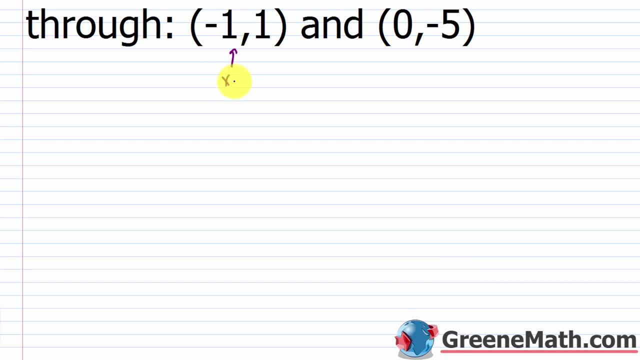 Again, let me calculate slope first. So I'm going to label this as x sub 1, y sub 1.. And this as x sub 2, y sub 2.. And then I'm plugging into my slope form. So m is equal to y sub 2 is negative. 5 minus y sub 1 is 1 over x sub 2 is 0 minus x sub 1 is negative 1.. 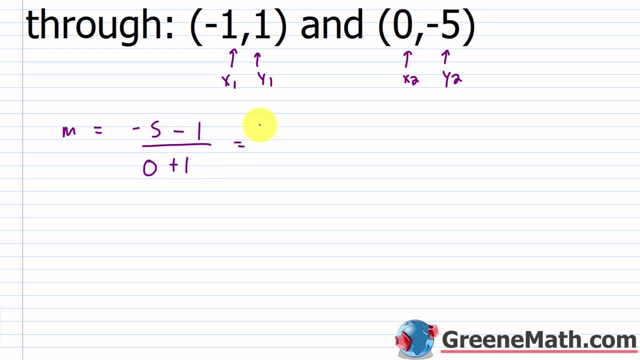 So minus a negative 1 is plus Negative. 5 minus 1 is negative 6 over 0 plus 1, which is 1.. So slope is just negative 6.. All right, m is negative 6 there. So now I plug into my point slope form. 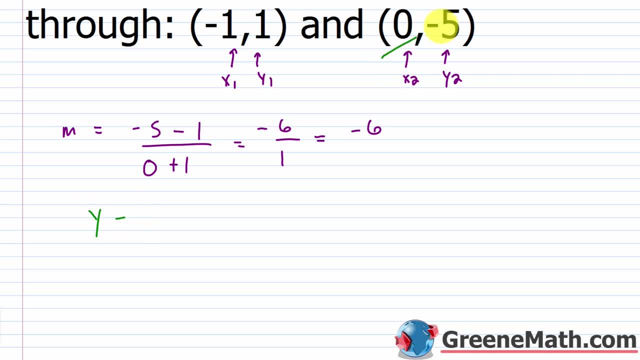 So y minus y sub 1.. And I can forget about this point now. I only need one of them, So let me just use this one. So let's say this is x sub 1, y sub 1.. So y minus 1 is equal to m, which is negative 6, times the quantity x minus x sub 1,. 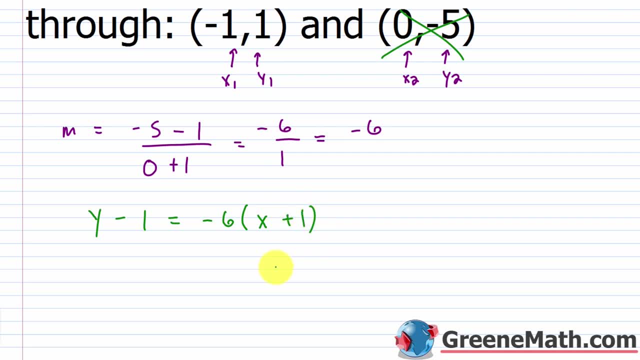 which is negative 6.. So y minus 1 is equal to m, which is negative 6, times the quantity x minus x sub 1, which is negative 1.. So minus a negative 1 is plus 1.. So now I'm going to solve this for y. 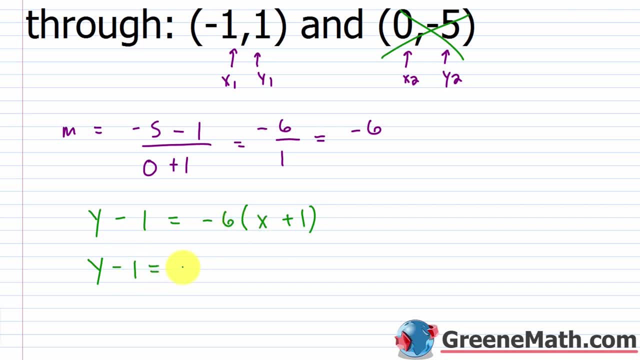 So let me say y minus 1 equals negative 6 times x is negative 6x. Negative 6 times 1 is minus 6.. Let's add 1 to each side of the equation And we'll get: y is equal to negative 6x. 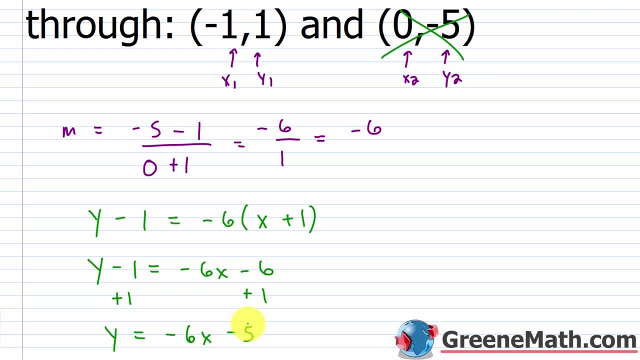 Negative, 6 plus 1 is minus 5.. So y equals negative 6x minus 5.. All right, let's take a look at one more. And then we're going to jump into standard form. All right, let's take a look at one more. 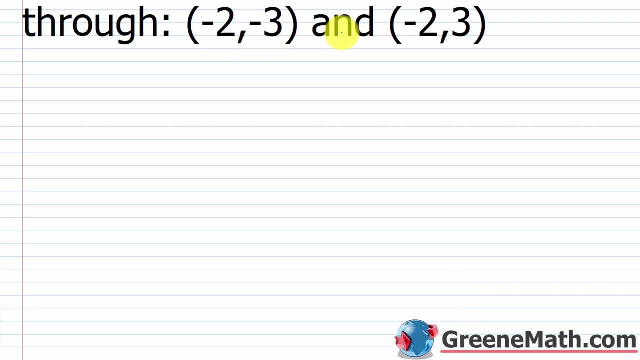 And then we're going to jump into standard form, So it passes through the point negative 2 comma negative 3, and negative 2 comma 3.. So some of you look at this and go: wait, something's wrong here. I've got negative 2 here and I've got negative 2 here. 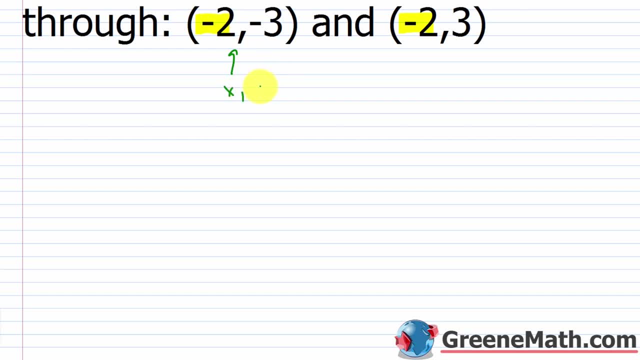 So if this is x sub 1, y sub 1, and this is x sub 2, y sub 2, what happens when I plug into the slope formula I get: m is equal to y sub 2 is 3 minus y sub 1.. 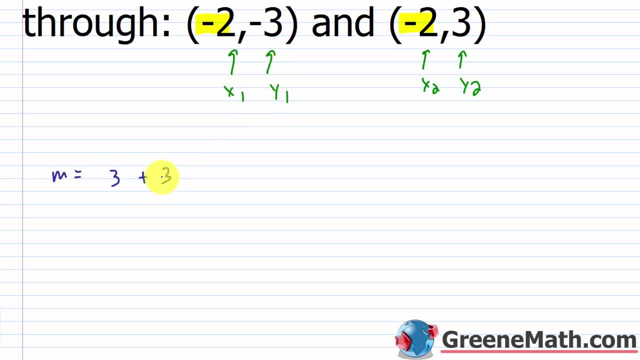 So minus a negative is plus 1.. Plus a positive, so plus positive 3.. Over x sub 2,, which is negative 2,. minus a negative, 2,, right Minus x sub 1,, so plus 2.. 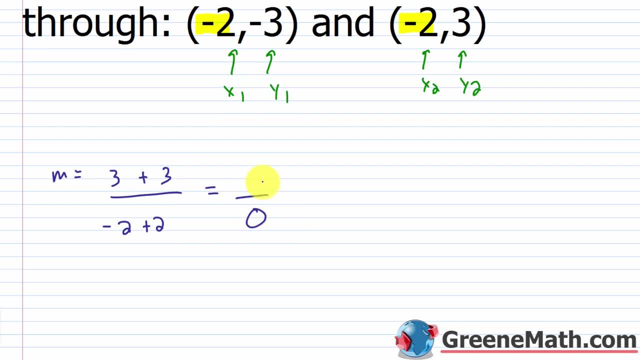 Well, the denominator here is going to be 0. Can't divide by 0, that's undefined. So this would be 6 over 0. This is undefined. What type of line has an undefined slope? Well, a vertical line does. 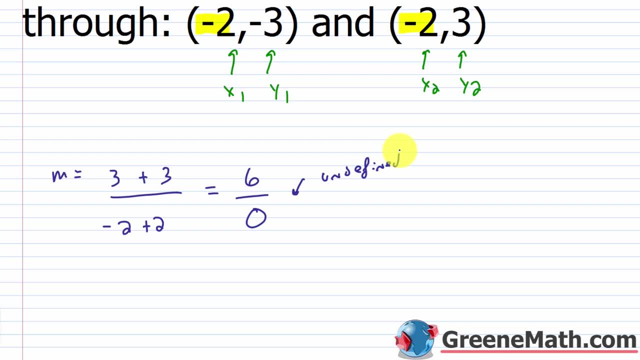 And that's x equals some number. So you can see that you have the same value for x here and here. So x is going to equal negative 2.. It's not hard to figure this one out. If I saw something where I had a horizontal line, I would have the same value for y in. 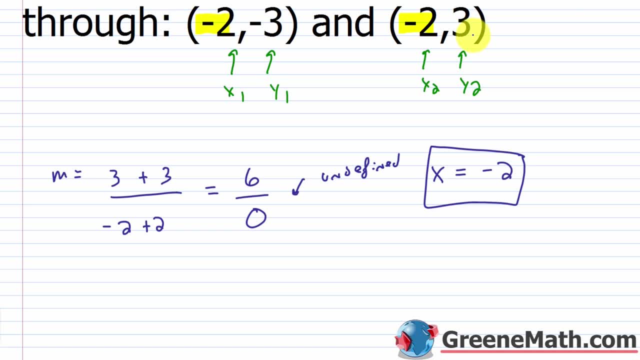 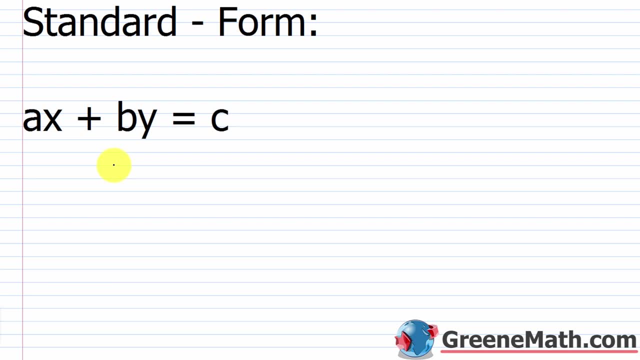 each case. If I have the same value for x in each case, I have a vertical line. All right, now let's talk about my favorite topic, because everyone wants to argue about it: the standard form. So standard form is going to vary from teacher to teacher, textbook to textbook, classroom. 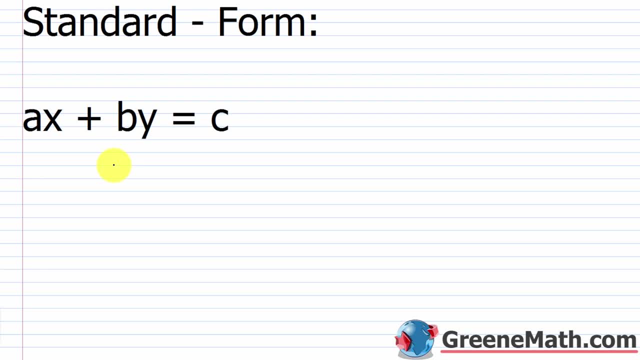 to classroom, High school to college, everybody says it's something different. okay, Let me give you the best definition I can for it. I'm going to tell you that standard form is where we write a linear equation in two variables where ax plus by equals c, like this, and a and b are not both 0. 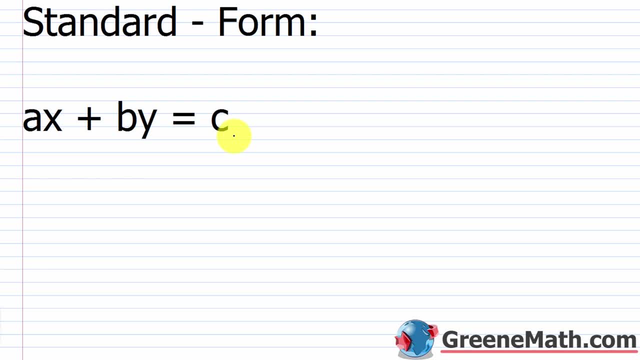 That's the definition you're going to use. if you're in high-level math, Nobody cares if there's integers or fractions or things like that. But For the time being, while you're in Algebra 2, while you're in high school, you're probably 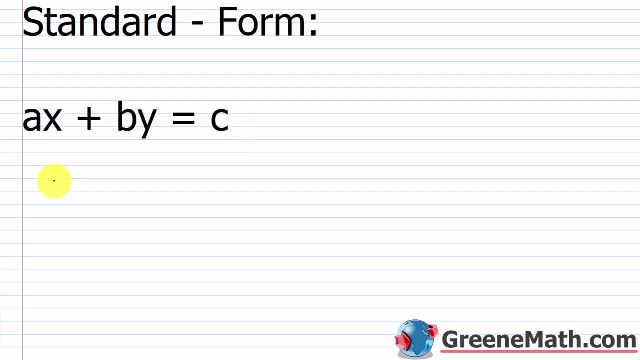 going to get a much stricter definition. You're probably going to be told that a, b and c are integers. so they don't want to see fractions, They don't want to see decimals, They don't want to see anything like that. 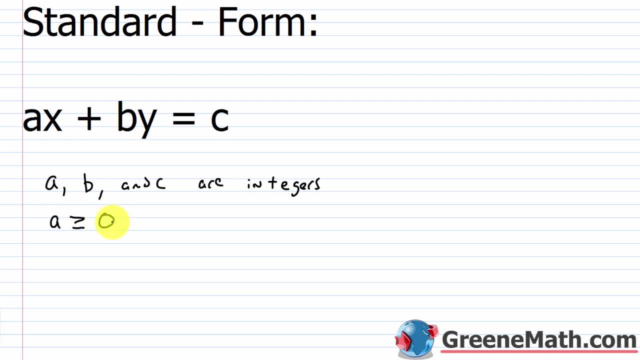 They're also going to tell you that a has to be greater than or equal to 0.. a and b are obviously not both 0.. And then, lastly, a, b and c have no common factor except 1.. Let's put: a, b and c have no common factor except 1.. 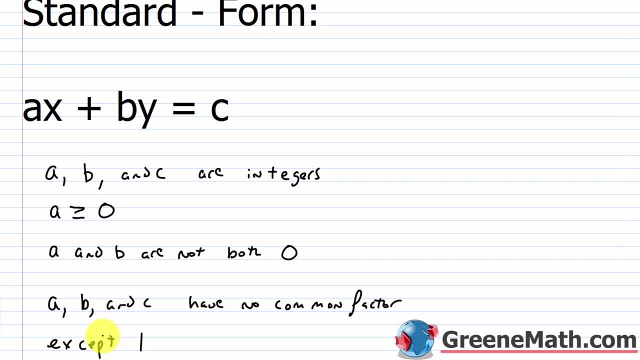 All right, so I would write this down. This is more than likely the case of what you're teaching. This is what your teacher wants you to do if you're in high school, If you're in a college Algebra course or something higher than that, and you're just watching. 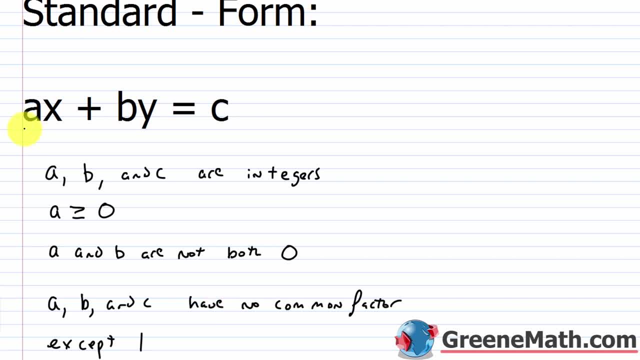 this to review. I wouldn't worry too much about it. You generally just use a, x plus b. y equals c. a, b and c can be real numbers. The reason we have a stricter definition in high school, or at least what I've been told. 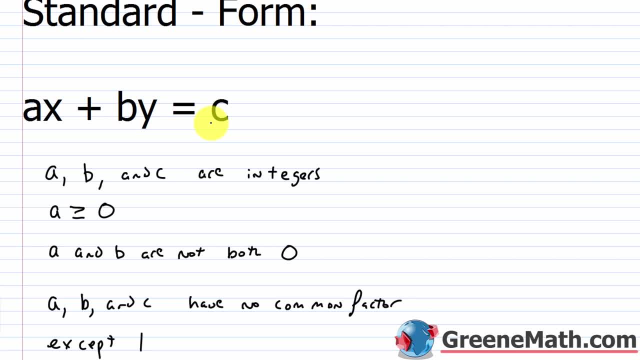 throughout the years is just to practice cleaning up equations. You get a lot of practice that you need Just manipulating things back and forth So that by the time you get into high level Algebra, this is not something that you struggle with. Another thing is it's going to help us have cleaner equations and ones that are more presentable. 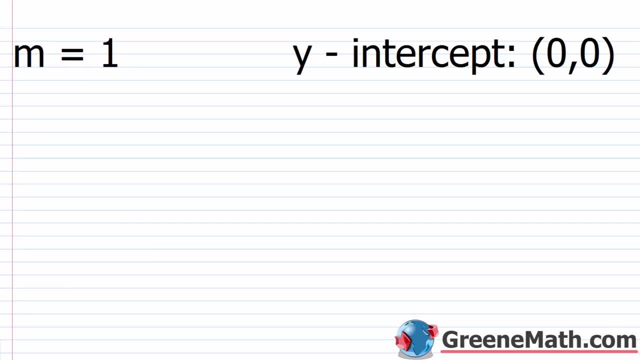 and easier to work with. So suppose I gave you this information and said: write an equation in standard form. So again, ax plus by equals c. Well, I know that the slope is 1, and I know the y intercept occurs at 0 comma 0. 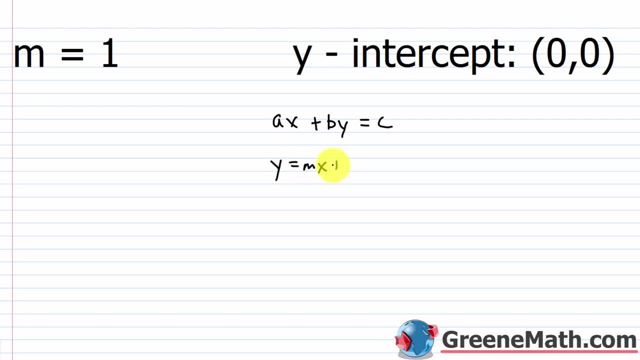 So I could start out with 1.. I'd have y equals mx plus b and I could put it in this format by doing some algebra: So y equals 1, which is my slope times x. so I'm just going to write x plus b here. 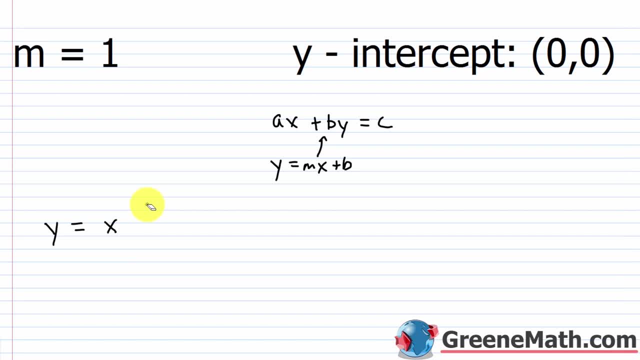 b is 0. So y just equals x. Well, this is easy. All I need to do is subtract x away from each side and I'd have negative x plus y equals 0.. Why is this in standard form? Well, again, it depends on whose definition you're using. 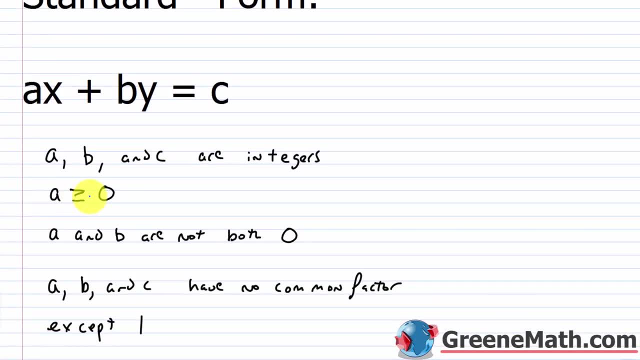 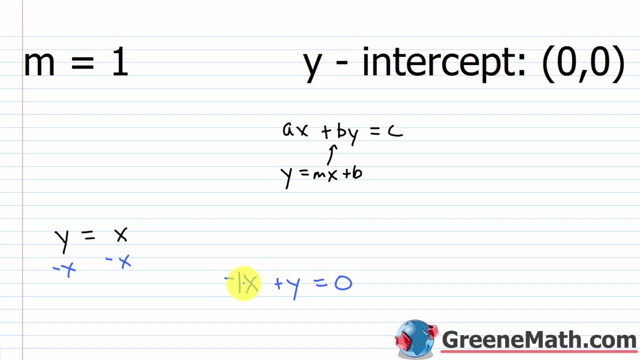 I told you, when I was kind of announcing this, that a needed to be greater than or equal to 0. In this particular case, I basically have a negative 1 as the coefficient for x. So in a stricter version you would say, no, this is not in standard form. 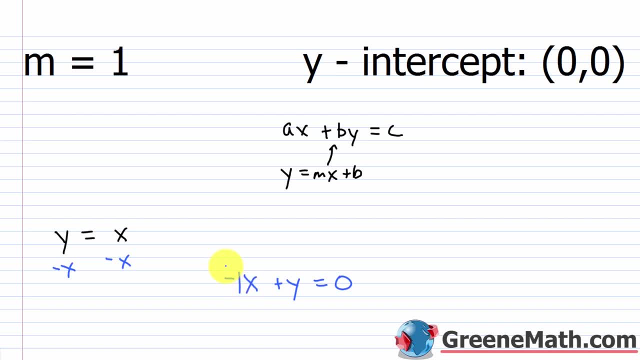 And all I would really need to do is multiply both sides of the equation by negative 1.. So if I do that, negative 1 times negative 1 is 1, so I just have x equal to negative, x plus y equals 0.. 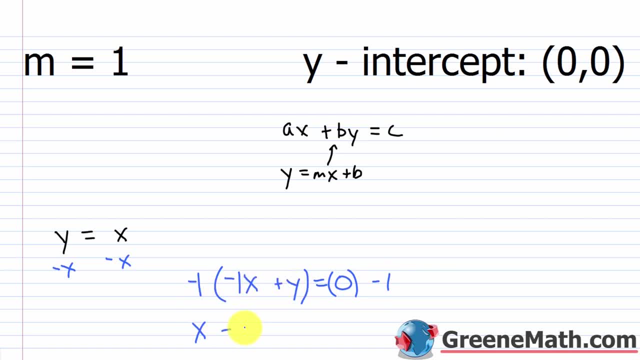 Really pushing this aside. Bye guys. x there Negative 1 times y is minus y And this equals 0 times negative. 1 is just 0. So I would have x minus y equals 0. And this is considered standard form, again, usually in a high school. 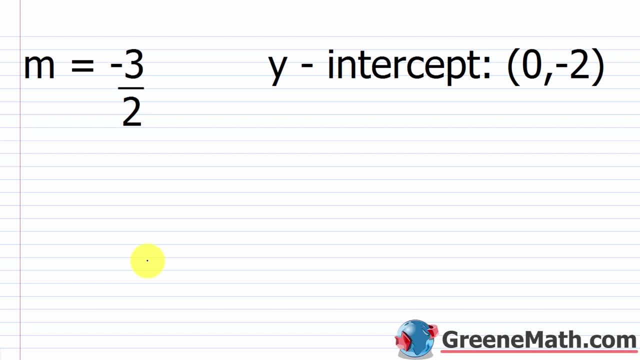 setting. All right, so the next one. we have a slope m that's equal to negative 3 halves and a y-intercept that occurs at 0 comma negative 2.. So again, if I write this in slope-intercept form, I'd have y equals negative 3 halves x and then minus 2.. Now I'm going to algebraically. 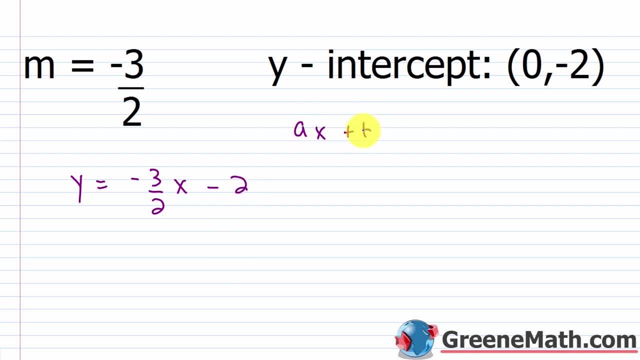 manipulate this. I want ax plus by equals c. So let me add 3 halves x to both sides of the equation And that's going to give me 3 halves x plus y equals negative 2.. Now there are some problems with this. 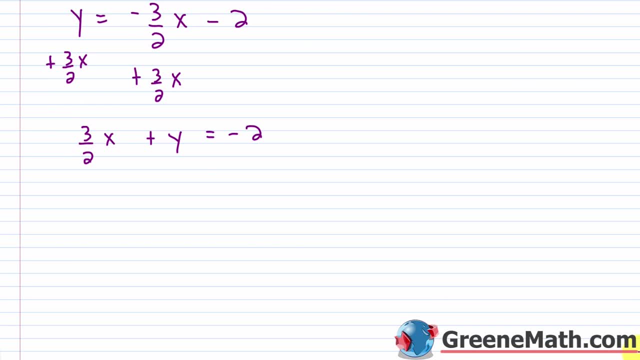 I want a, b and c to be integers. Right now my a is a fraction, So how can I deal with that? Well, I just multiply both sides of the equation by 2, and I clear the denominator. So 2 times 3. 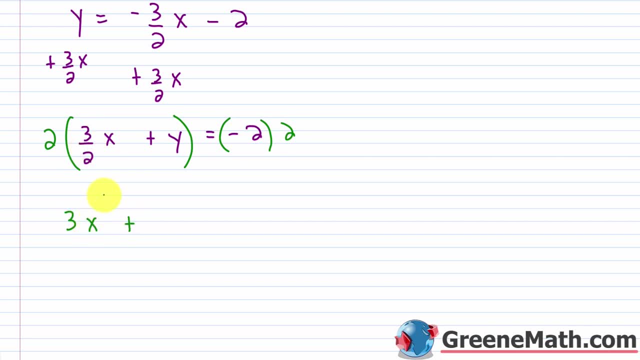 halves is 3.. So this would be 3x plus 2 times y is 2y, And this equals 2 times negative 2 is negative 4.. So now I've met all the requirements. This is greater than or equal to 0, so that's okay. 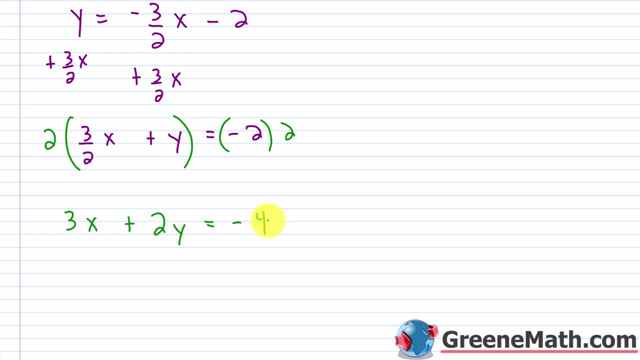 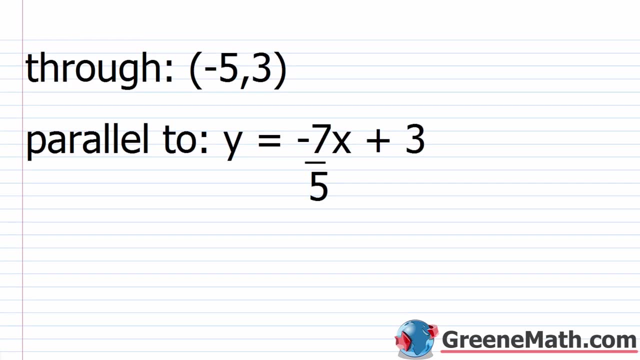 a, b and c are integers, so that's okay, And there's no common factor between the three- a, b and c- other than 1.. All right, so now we want to look at something a little bit more complex. We still want to. 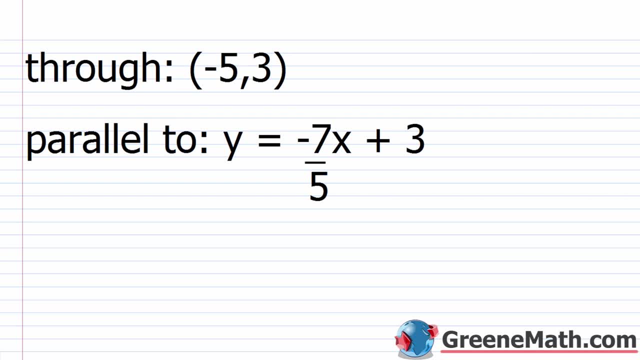 write it in standard form, but the information gets a little trickier. It's through this point: negative 5 comma 3, parallel to y, equals negative 7 fifths x plus 3.. So if I have it, I have a point and I have the slope. I can write it in point-slope form, as we learned. 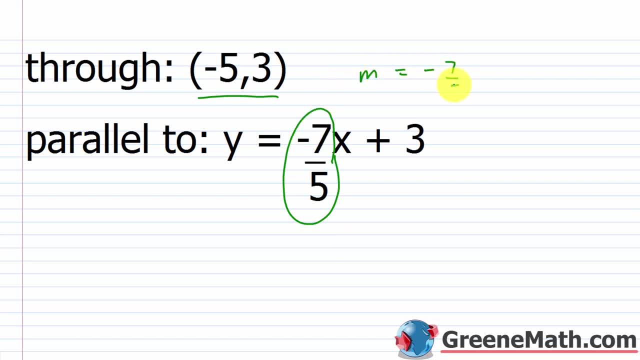 a little while ago. So m here would equal negative 7 fifths. Now, once I extract the information from this equation here, I don't need it anymore- Cross it out. It's going to confuse you. You don't need it, So get rid of it. Now I want to plug in a point-slope. 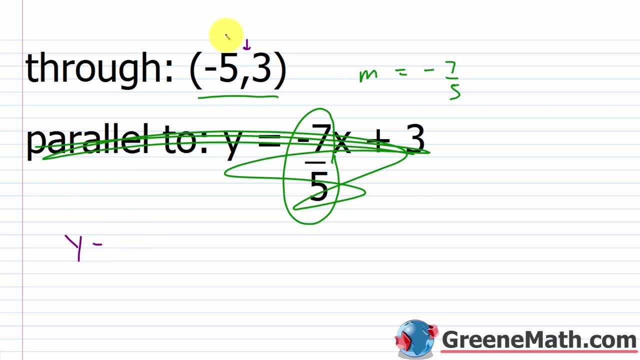 form, So y minus. if I label this as x sub 1, y sub 1, then y sub 1 is 3. This equals m, which is negative 7 fifths times the quantity x minus x sub 1 is negative 5.. 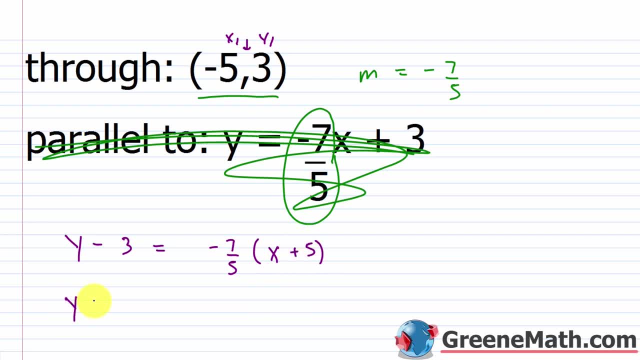 So minus the negative 5 is plus 5.. So I'd have: y minus 3 is equal to negative 7 fifths times x is negative 7 fifths x. Negative, 7 fifths times 5, the 5s are canceled. 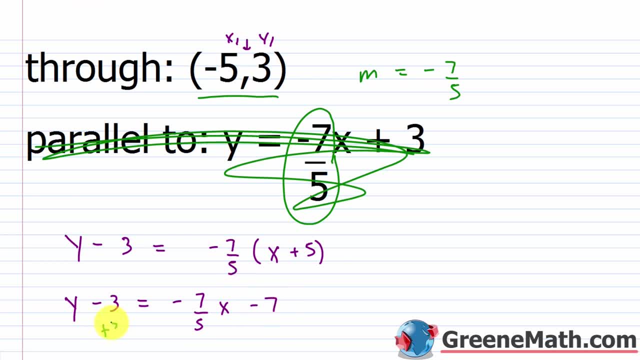 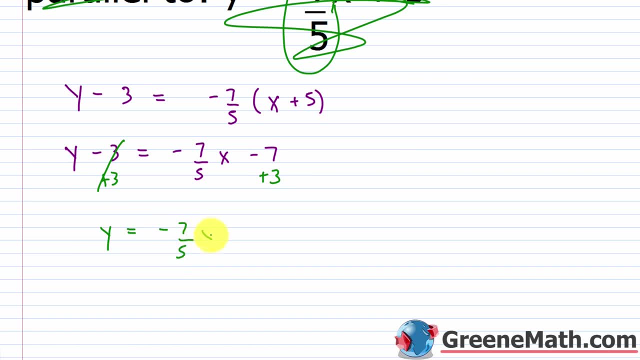 You'd have minus 7.. So now, if I add 3 to each side, this will cancel. I'll have: y is equal to negative 7, fifths x Negative. 7 plus 3 is negative 4.. So now I have it in slope-intercept form, but I want it in standard form. 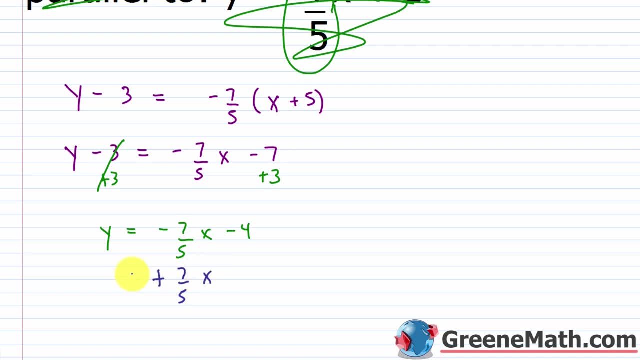 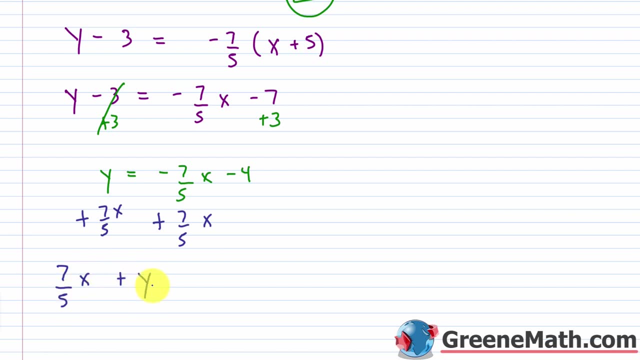 So let me add 7 fifths x to both sides of the equation And what I'm going to have is 7 fifths x plus y is equal to negative 4.. So, as a final step- remember, I don't want this to be a fraction- 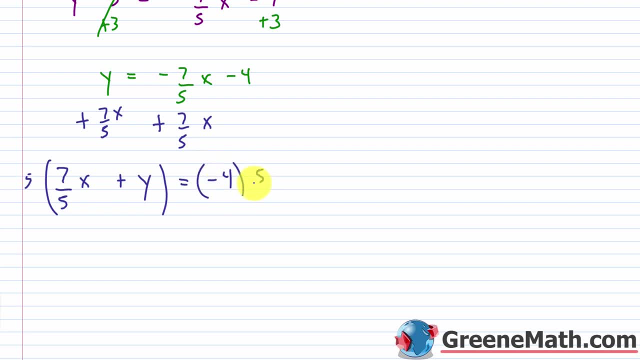 So I'm going to multiply both sides of the equation by 5 to get rid of that. 5 times 7, fifths is 7.. So 7 times x or 7x plus 5 times y, is 5y is equal to negative 4 times 5, which is negative 20.. 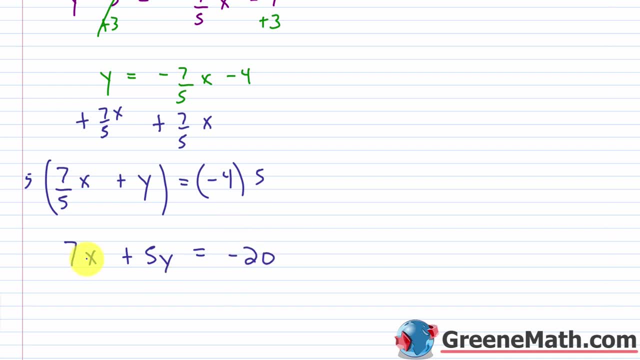 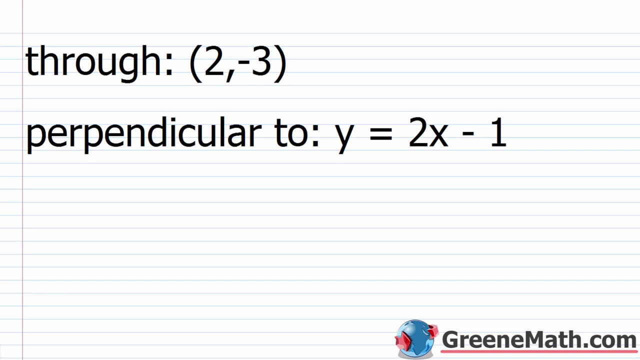 So in standard form this equation is: 7x plus 5y equals negative 20.. All right, let's take a look at one more. So perpendicular lines have slopes where the product would be negative 1.. So 2 times what equals negative 1?. 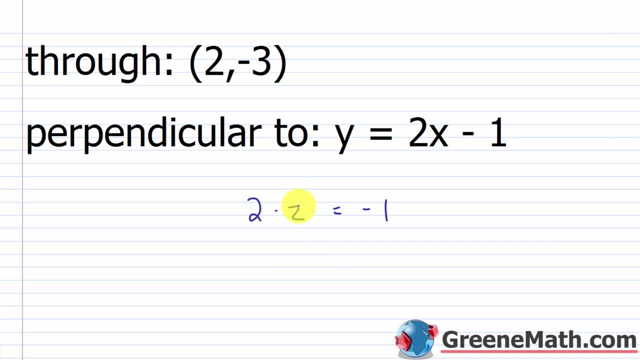 Well, you could use a variable. Let's say z is such a number that you're looking for. Divide both sides by 2, and you're going to find that z, or your unknown number, is negative 1 half. So that's the slope that you would have. 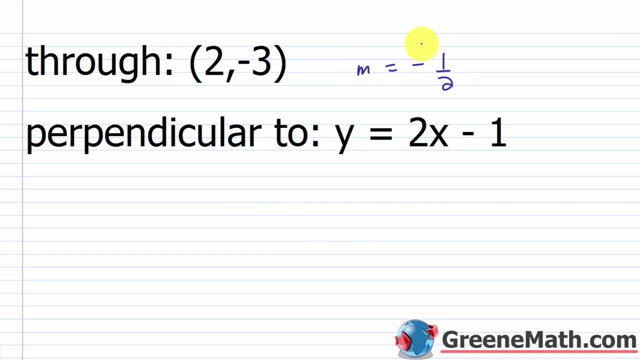 m here would be negative 1 half again, because negative 1 half times 2 would give you negative 1. And perpendicular lines have slopes whose product is going to be negative 1.. So again, once you've used this, get rid of it. 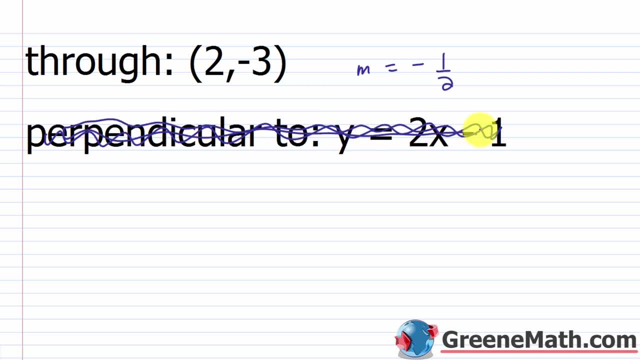 Don't want to think about it anymore. It's not relevant to anything else. So now, if this is x sub 1.. y sub 1, I'm going to plug into my point slope form. So y minus or y sub 1, I've got negative 3, minus. the negative 3 is plus 3, equals m. 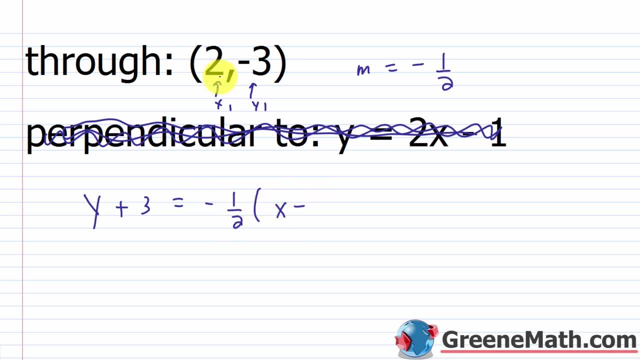 which is negative 1 half times the quantity x minus for x sub 1, I have 2.. So I have: y plus 3 is equal to negative 1 half times x is negative 1 half x, Then negative 1 half times negative 2, the negatives would cancel. 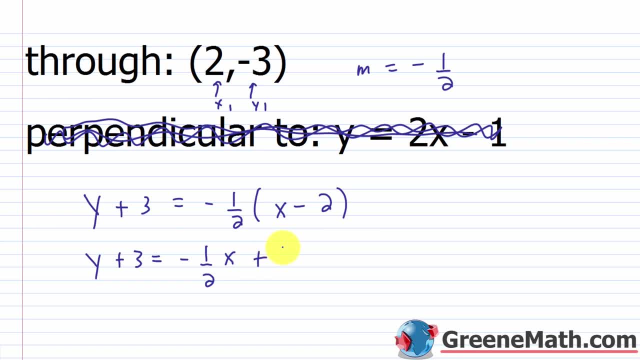 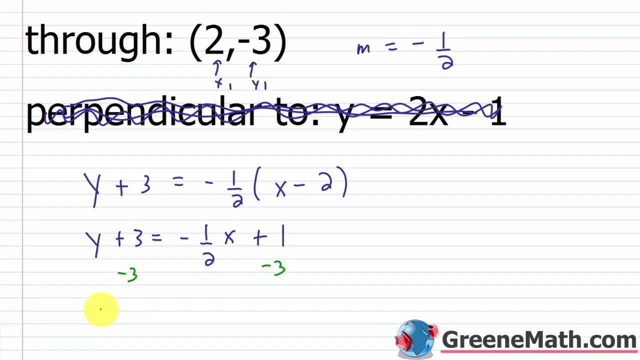 That would be positive. 1 half times 2 is negative. 1 half 2 is 1.. So now I'm going to just subtract 3 away from each side of the equation. I'll have: y is equal to negative. 1 half x. 1 minus 3 is negative 2.. 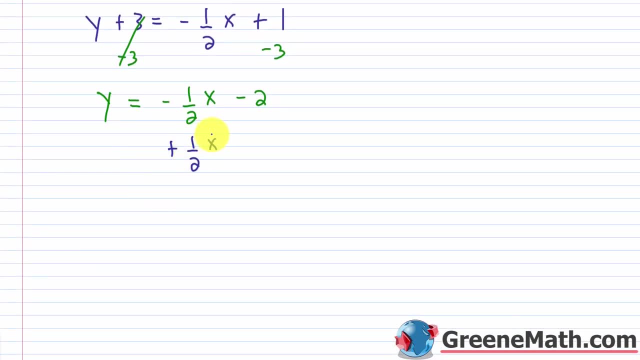 All right, The last thing I'm going to do is add 1 half x to each side of the equation, So I'll have 1 half x plus y is equal to negative 2.. And then I want to clear this. Clear this fraction, right. 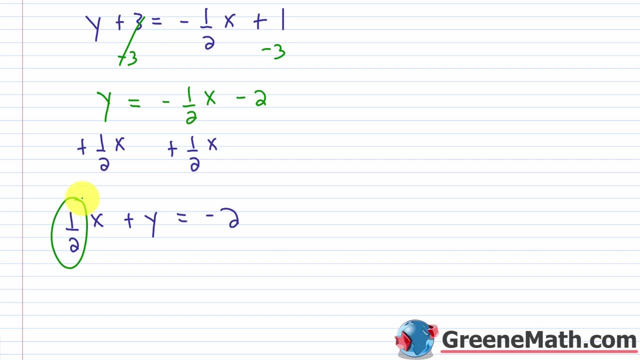 I don't want that, So to do that, I'm just going to multiply both sides by 2.. Multiply this side by 2.. Multiply this side by 2.. 2 times 1 half is 1.. So it's just x. 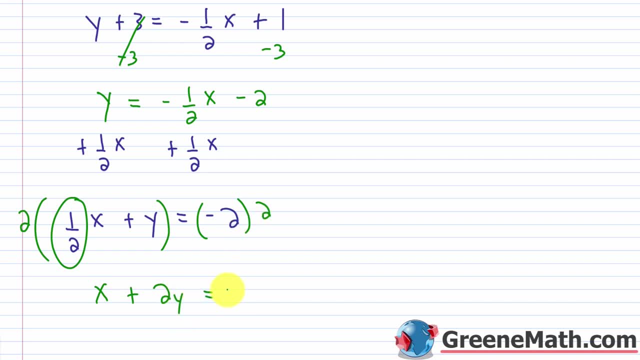 Plus 2 times y is 2y And this equals negative 2 times 2,, which is negative 4.. So finally, I have this in standard form. I have x plus 2y equals negative 4.. Hello and welcome to Algebra 2, Lesson 20.. 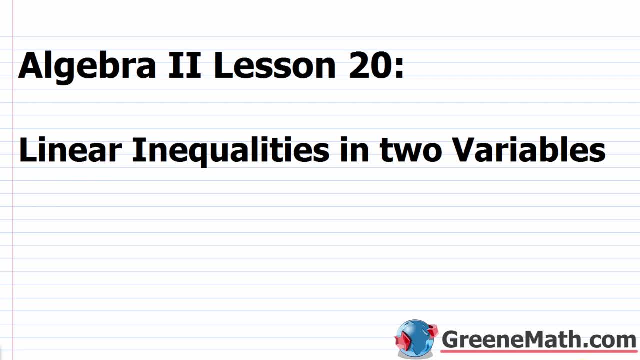 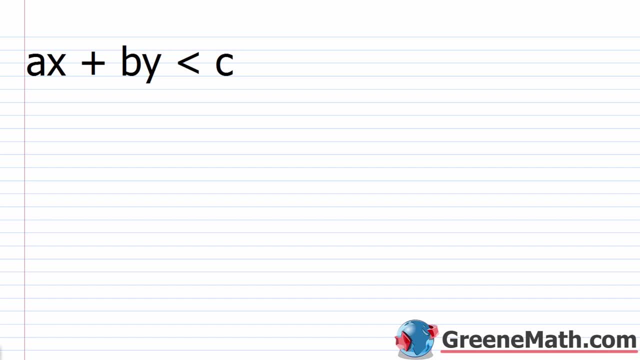 In this video we're going to learn about linear inequalities and we're going to learn about linear inequalities in two variables. So once we've mastered the art of graphing a linear equation in two variables, you're going to find that it's not much more difficult. 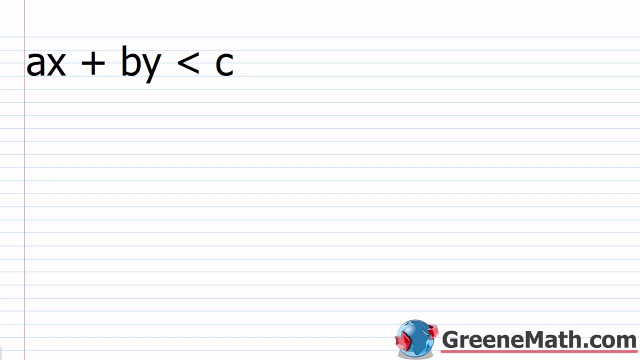 to master the art of graphing a linear inequality in two variables. So we start out with a basic form. This is something you'll see in your textbook. So a linear inequality in two variables is of the form: ax plus by is less than c. 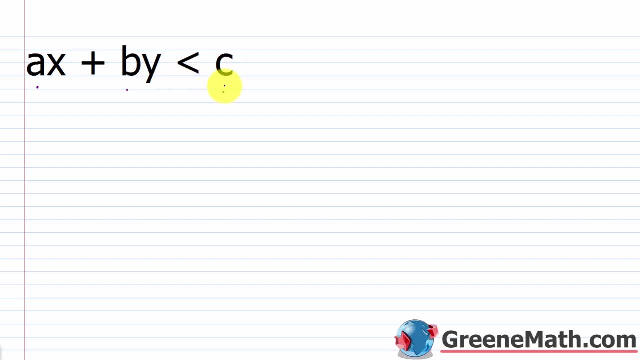 where we would say a, b and c are real And then a and b are not both zero. Now also this less than symbol here could be a greater than, it could be a less than or equal to, or it could be a greater than or equal to. 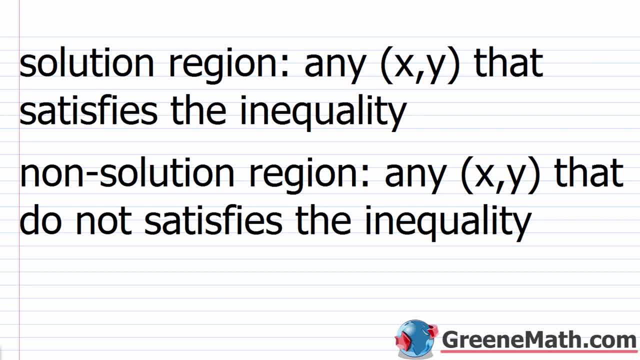 Now, when we talk about graphing a linear inequality in two variables, when we look at our coordinate plane, it's going to have three distinct regions. So the first region I'm going to talk about is the solution region. So this is where we have any ordered pair. 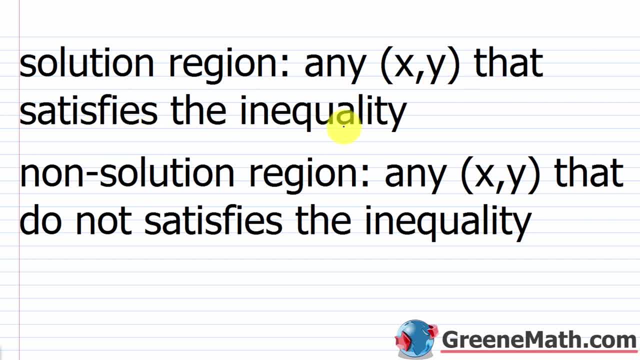 So we have x- y. that satisfies the inequality. The next part I would talk about is the non-solution region. So this is any x, y or any ordered pair that does not satisfy the inequality. So you have two separate regions. Now these regions are separated by something known as a boundary line. 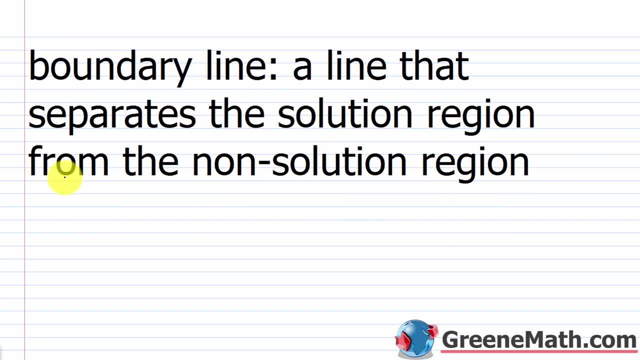 So the boundary line is a line that separates the solution region from the non-solution region. Now, the key thing to understand here is that this boundary line can be part of the solution or it can be not part of the solution. It's based on what type of inequality you get. 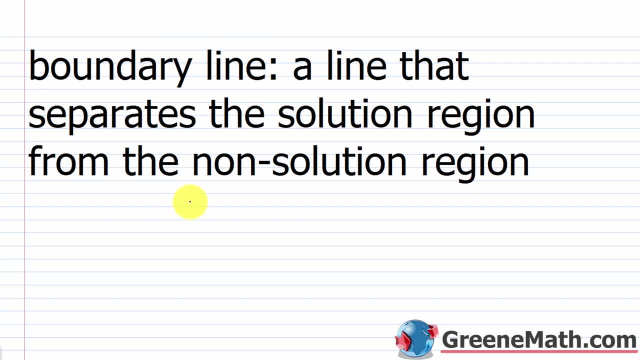 If you get a strict inequality, meaning you get a greater than or a less than- this is strict- then the boundary line is not part of the solution. If you get a non-strict inequality, meaning you have greater than or equal to, or less than or equal to, 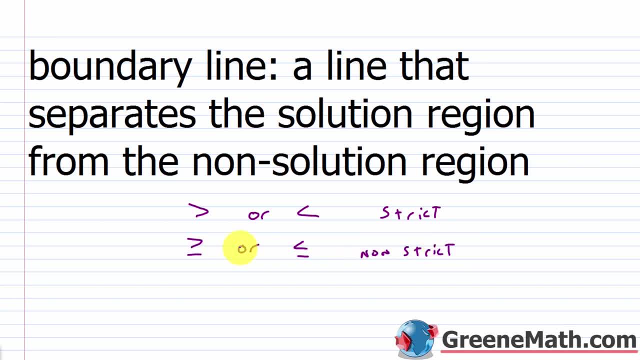 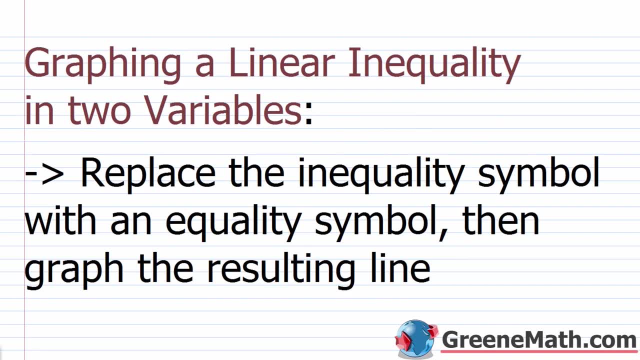 this is non-strict, then in this particular case, your boundary line is part of your solution. All right, so let's talk a little bit about how we actually go about doing this. It's quite similar to again graphing a linear equation to variables. 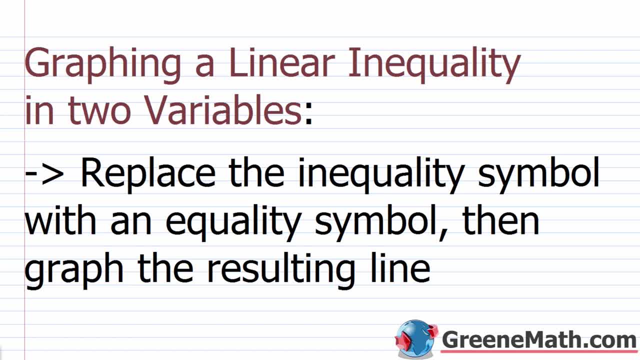 with just a little bit of a twist to it. Now, there's two kind of ways to do this. One way is a little bit slower, to involve something known as a test point, And then the other way involves just solving for y. So I'm going to go through both procedures for you. 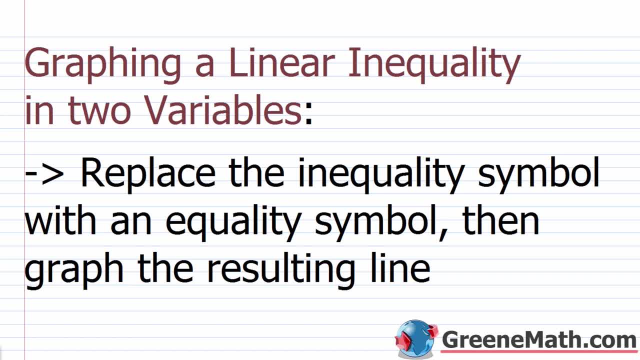 And then you can choose which one is better for you. So graphing a linear inequality in two variables. The first thing we want to do is replace the inequality symbol with an equality symbol, then graph the resulting line. This is how we get the boundary line okay. 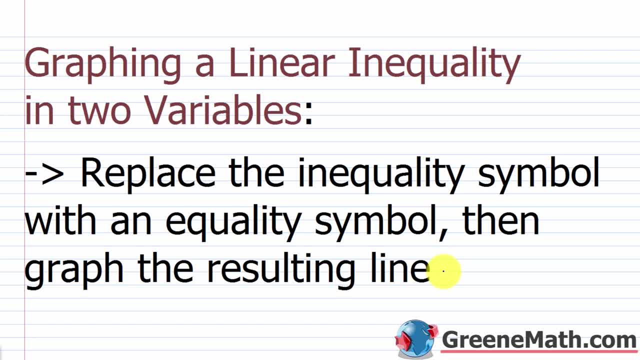 When we do this. if the inequality symbol again is strict, then we want a dashed line, because the boundary line in that case is not part of the solution. If the inequality is non-strict, we want a solid line, because in that case the boundary line is part of the solution. 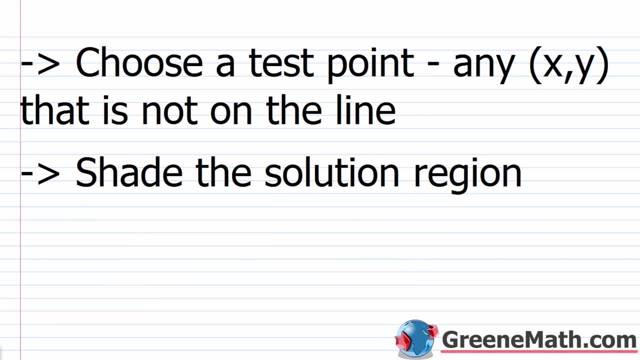 Now the next thing we want to do is we want to choose a test point. So this is any ordered pair that is not on a line. So you just plug it back in to the original inequality and you see if it works. So if it does work, you're in the solution region. 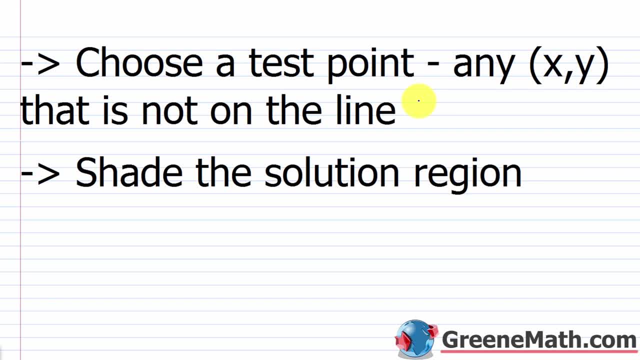 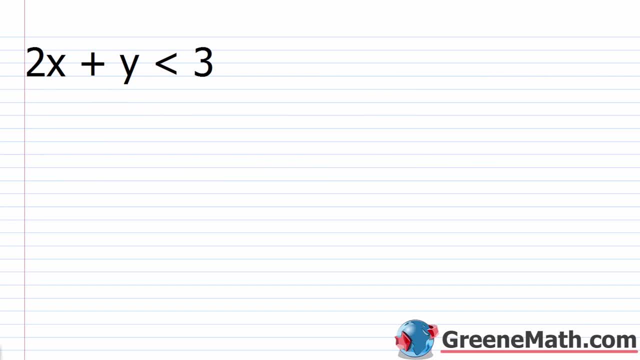 So you shade that region where the test point is. If it doesn't work, then you're in the non-solution region and you just shade the other side, All right. so let's start out with the first example We have: 2x plus y is less than 3.. 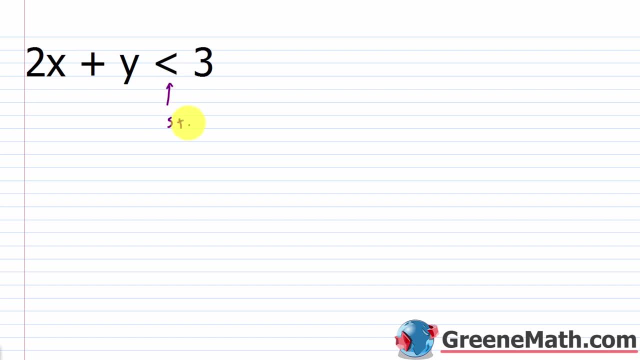 So the first thing I want to call your attention to is that this is a strict inequality. So that tells me that my boundary line is going to be not part of the solution, and so I want a dashed line. Usually what I do is I'll take and draw either gaps in my line. 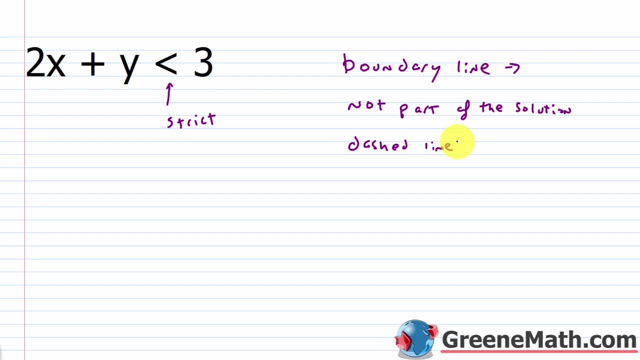 or I'll draw a solid line and then kind of erase it, depending on what method I'm drawing with. If I'm on a computer, then I'm going to break it up. If I'm drawing with a pencil, then I'll just kind of gap it. 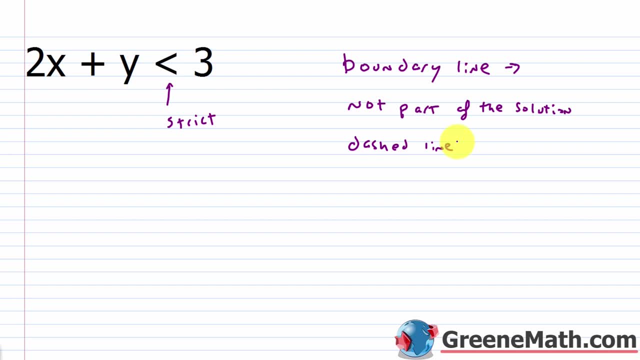 So we have a strict inequality. The boundary line is dashed or broken. Now, the other thing I would call your attention to is that it's not solved for y right now, and I'm going to get to that in a minute. So all I'm going to do is I'm going to replace this with equals. 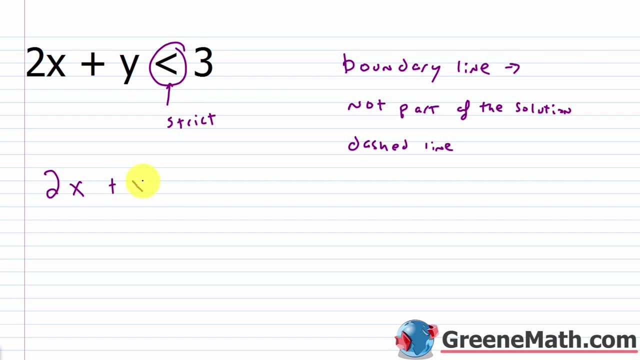 So I'm going to pretend like I have: 2x plus y is equal to 3.. I'm just going to graph this. This is going to be my boundary line. This is the boundary, So this will separate the solution region from the non-solution region. 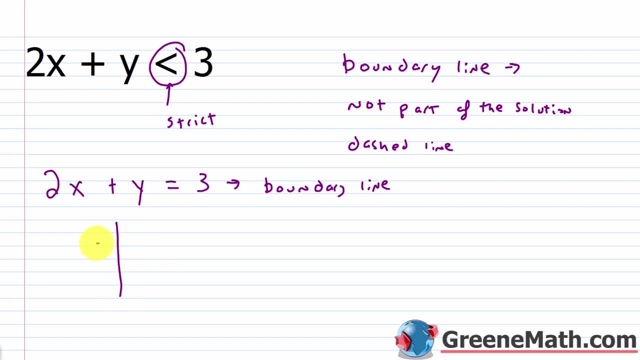 Okay, so we know how to graph this. Let's get some points going. So, if x is 0, y is 3.. If let's say, I don't want to use the x intercept because that's going to give me a non-integer. 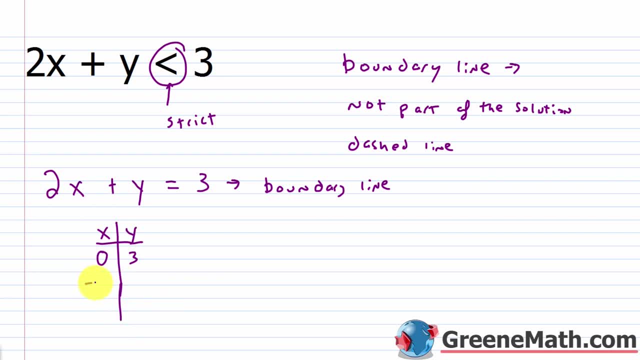 But let's go ahead and say: if x was negative, 2, I would have 2 times negative. 2 plus y equals 3.. So this would be negative. 4 plus y equals 3.. Add 4 to each side and I get y is equal to 7.. 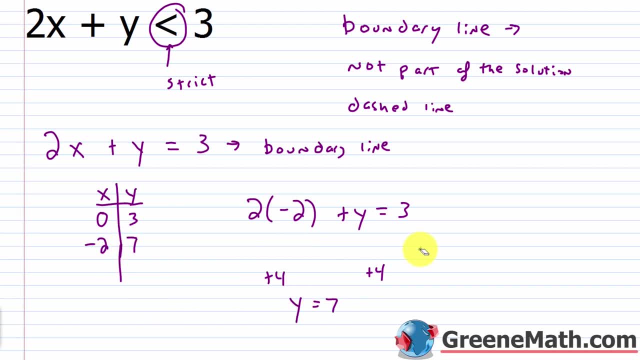 So if x is negative, 2,, y is 7.. And let me get one more point going here. Let's say x is positive 2. So I'd have 2 times 2,, that's 4, plus y equals 3.. 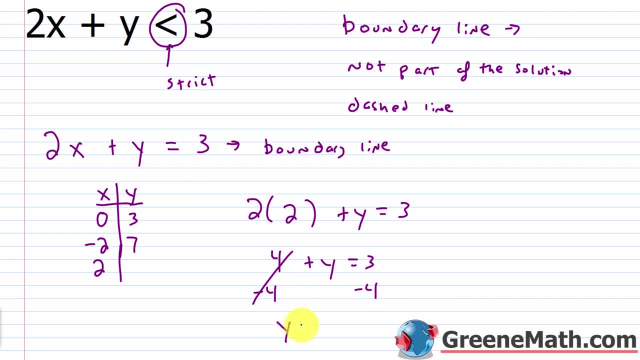 Subtract 4, away from each side of the equation I'd have, y is equal to negative 1.. So I have 3 points there, 3 ordered pairs, And I'm just going to plot them on the coordinate plane. So 0 comma 3, negative 2 comma 7, and 2 comma negative 1.. 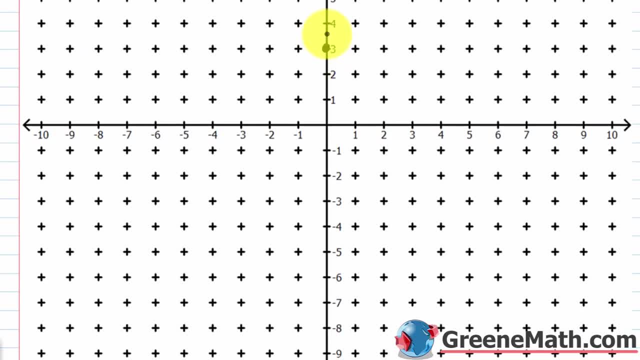 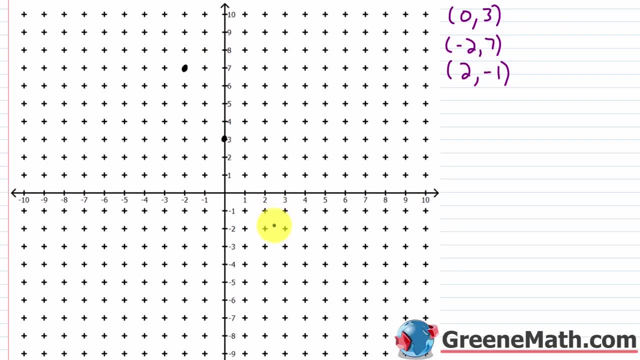 So 0 comma 3, that's going to be right here. Negative 2 comma 7.. So I go 2 units to the left, 7 units up, that's right here. And then 2 comma negative 1, so that's going to be right here. 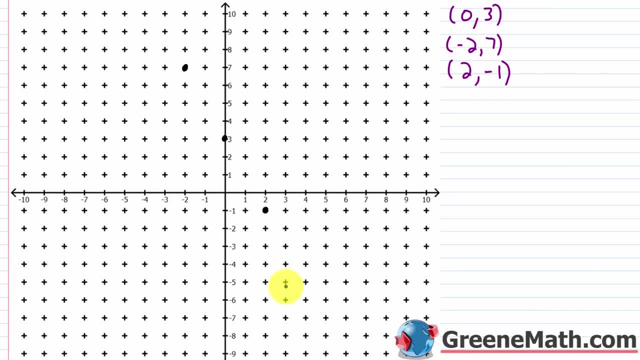 So again, this line that I'm going to draw right now should be broken or dashed. So because I'm drawing this on a computer, I'm just going to draw a straight line, then use an eraser to break it up, OK. 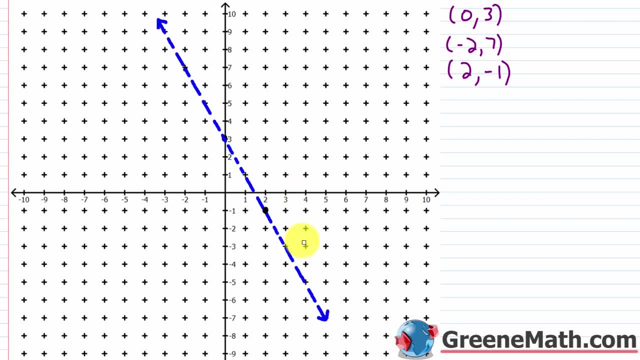 And then let me get my eraser. OK, that should be good enough. So you just want to make it obvious that you have a broken up or dashed line. Again, a broken line means that the line is not part of the solution. 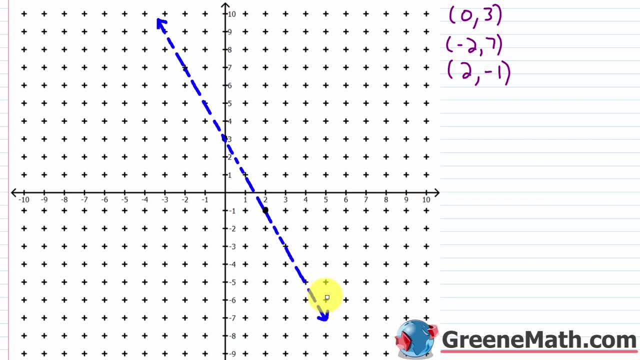 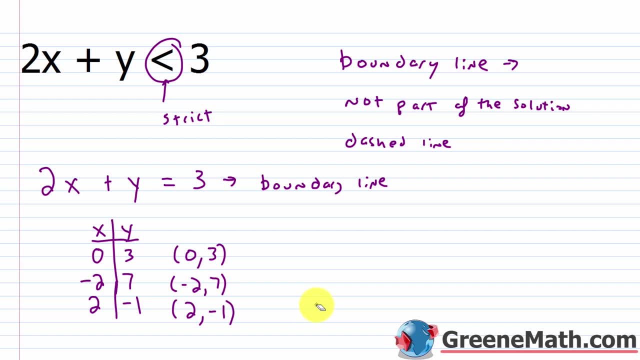 If you have a solid line, it is part of the solution. And I'll give you an example of this. If I take 0 comma 3, let's go back up And I plug that in Because 0 comma 3 is on the line. 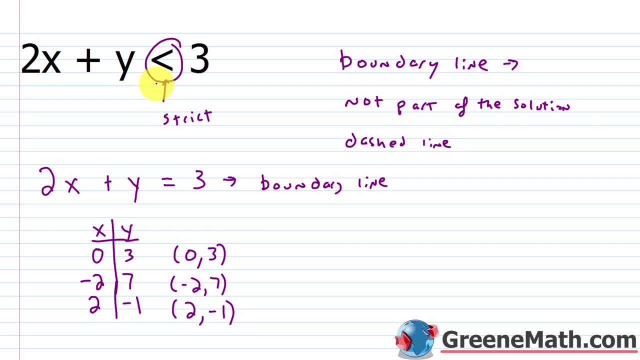 and this is a strict inequality. it should not work. So let's see if it does. So we have: 2 times 0 plus 3 is less than 3.. 2 times 0 is 0, so this would cancel. 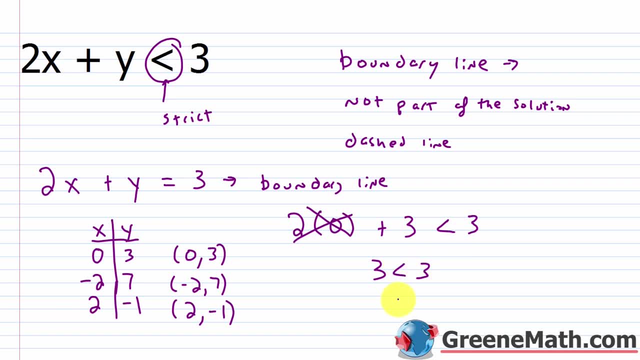 You'd be left with: 3 is less than 3.. Well, that is not true. 3 is not less than 3.. 3 is equal to 3.. But if this was a non-strict inequality, let's say, for example, I had less than or equal to over here. 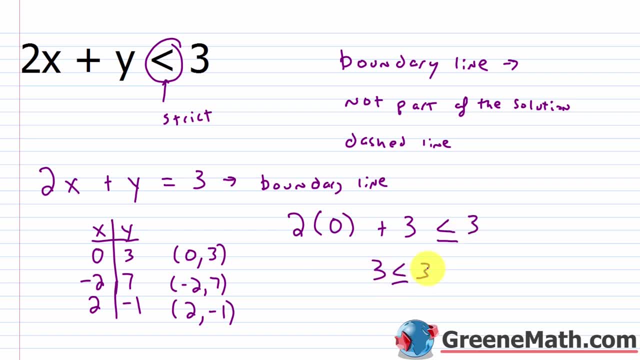 Well then, if it gets to this, 3 is less than or equal to 3, well, that would work. So you can see that your boundary line is part of the solution if you have a non-strict inequality, but not part of the solution if you don't. 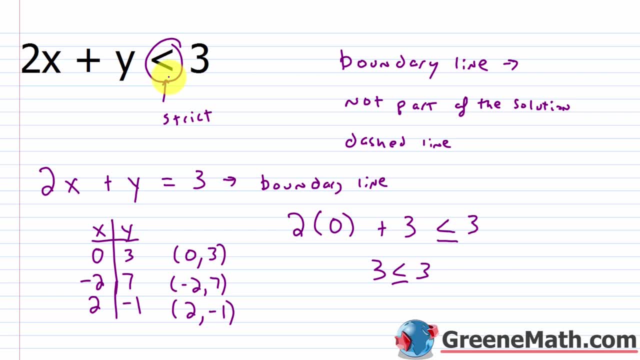 So in this case, we've got a strict inequality, so it's not part of the solution. Now, the next thing we want to do is we want to choose a test point. So let me go back to the coordinate plane. You want to look for something that is not on the line. 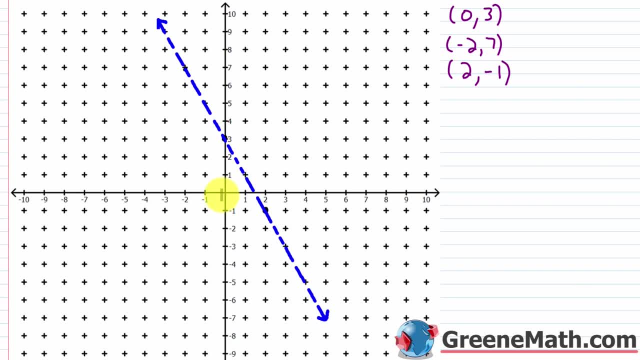 The most common test point you'll use is 0, 0, because it's nice and easy to work with. So you're going to say: is 0, 0 a solution for that inequality? If it is, I'm going to shade everything in that region. 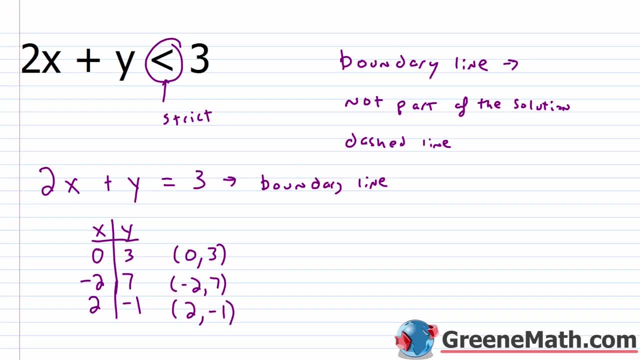 If it's not, I'm going to shade everything in the other region. So I go back up here and I say my test point is 0, 0. So I just plug it. So I say 2 times 0 plus 0 is less than 3.. 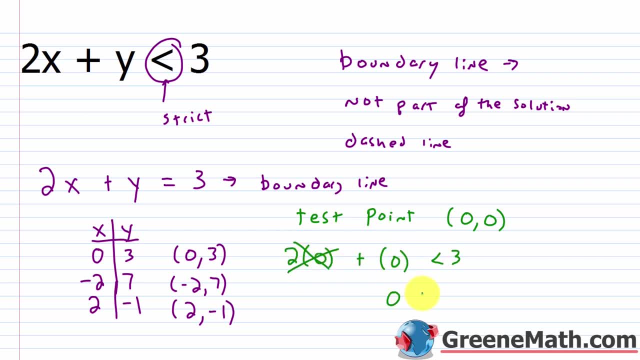 2 times 0 is 0, so that's gone. Plus 0 is 0. So you would get: 0 is less than 3.. That's true. So if this is true, that means that 0, 0 lies in the solution region. 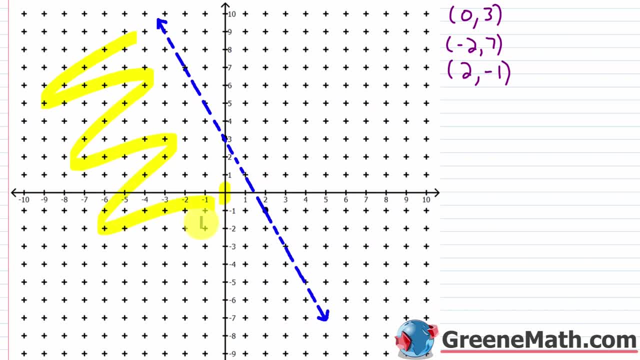 So that means that everything over here satisfies the inequality and everything on the other side of the boundary line does not, And you could choose a test point over here and see if it doesn't work. So something like, let's say, 4 comma 1.. 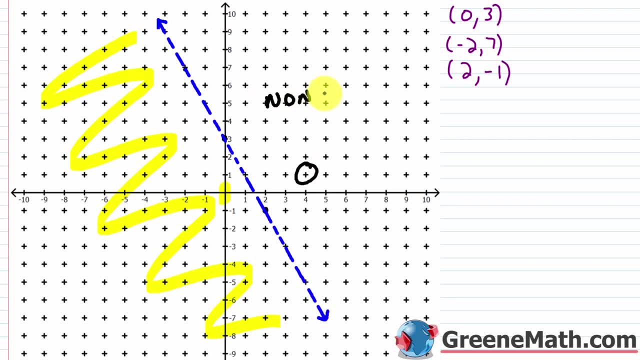 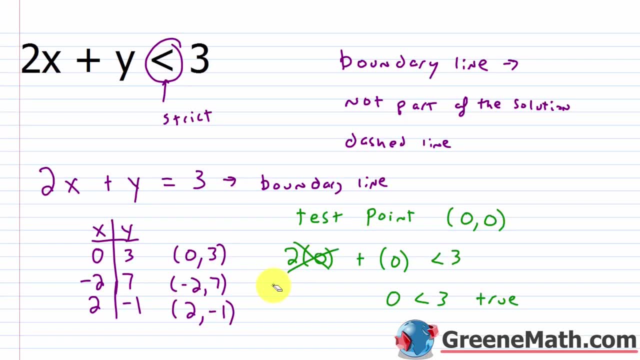 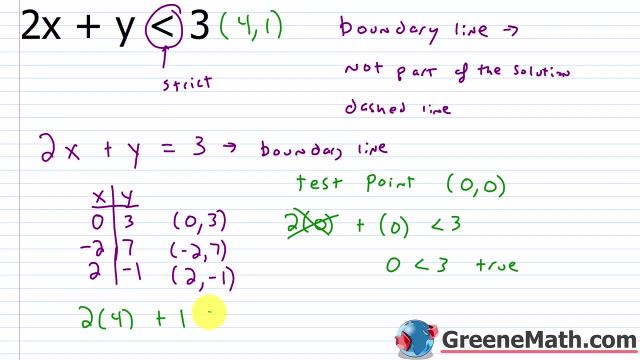 So this is in the non-solution region. Non-solution region And let's say we look at 4 comma 1.. So I would have: 2 times 4 plus 1 is less than 3.. 2 times 4 is 8.. 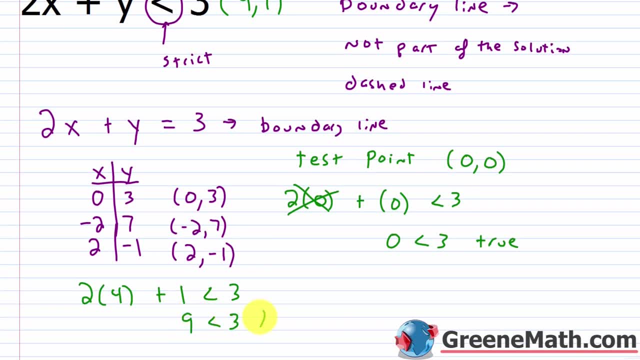 8 plus 1 is 9.. 9 is not less than 3.. So this is false. And we expect it to be false because I took a point that was in the non-solution region. It should not work and it didn't. 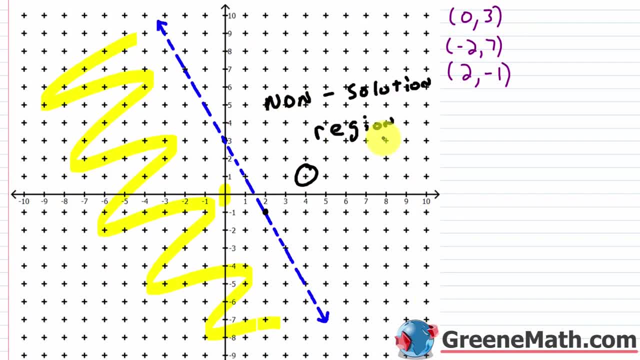 So that's good, But when we look at this again, this is the non-solution region. Over here is the solution region. So typically we will shade this And, depending on what you're working with, if you're in class you don't have a computer. 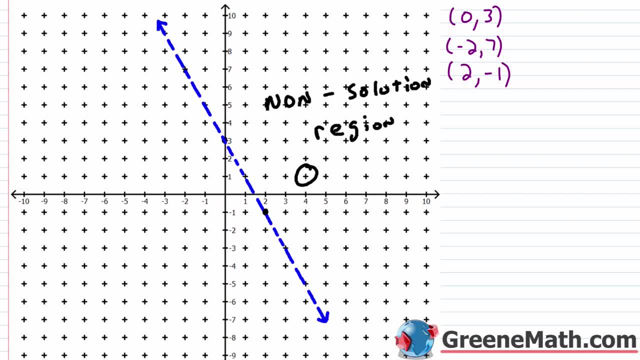 you would just kind of shade in the direction of the solution region. So I'll show you this. I'll just take a black marker and just shade here, Put arrows at the end to say, hey, this continues forever in this direction. Anything on this side of the line. 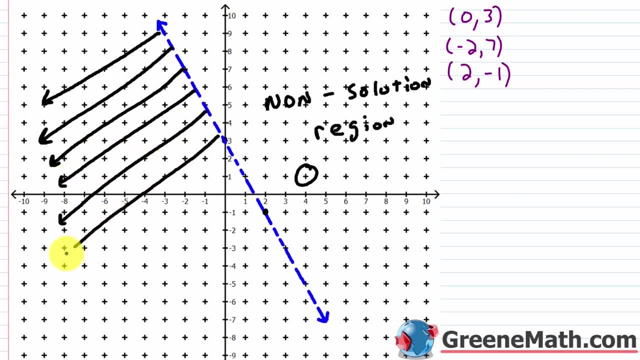 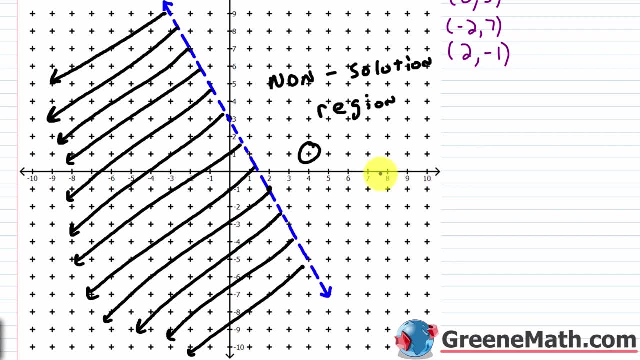 would satisfy that linear inequality in two variables. So again you can see three distinct parts: Non-solution region, boundary line, which in this case is not part of the solution, and then your solution region. Three parts. Now let me talk a little bit about. 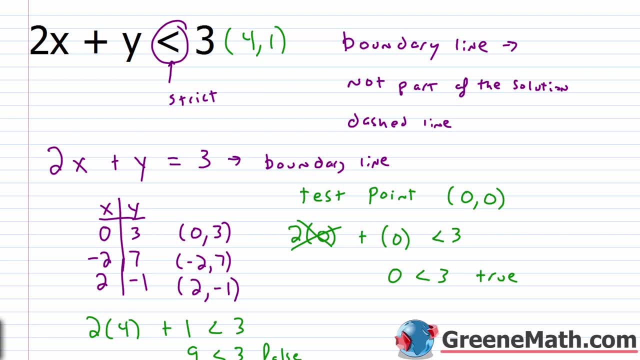 how to do this in what I would say an easier fashion. So let's erase everything here Now. some textbooks will cover this, Others will not, And again, it's a matter of personal preference. I don't like using a test point. 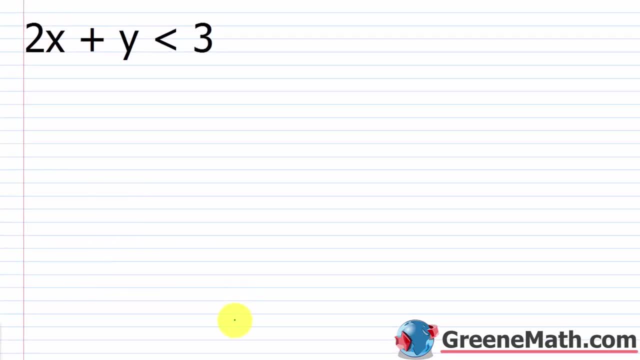 I just think it's very slow. What I do personally, and what a lot of teachers will have you do, is just start out by solving the inequality for y. So remember, if you have an equation solved for y, it looks like this: y equals m, the slope times x plus b. 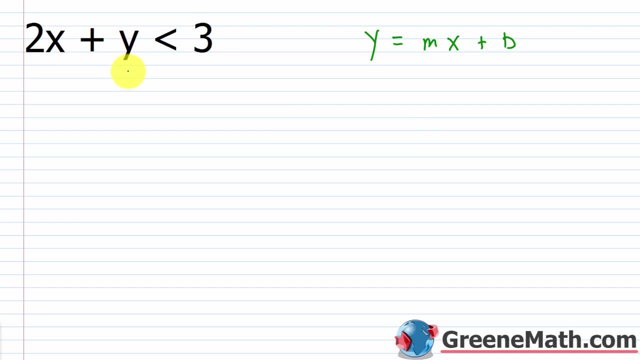 And this particular equation is an inequality, but we're going to just put it in this format. So I'm going to subtract 2x away from each side. I'll have: y is less than negative 2x plus 3.. Now I'm going to replace this: 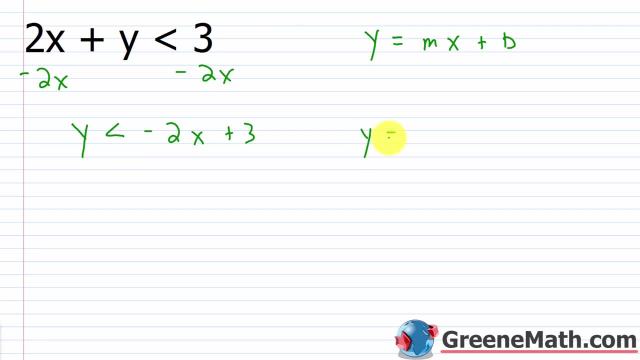 with an equality symbol. So I'm going to have: y is equal to negative 2x plus 3.. And I'm still going to draw my boundary line. This is still the boundary And it's still going to be a dashed line, because this is strict. 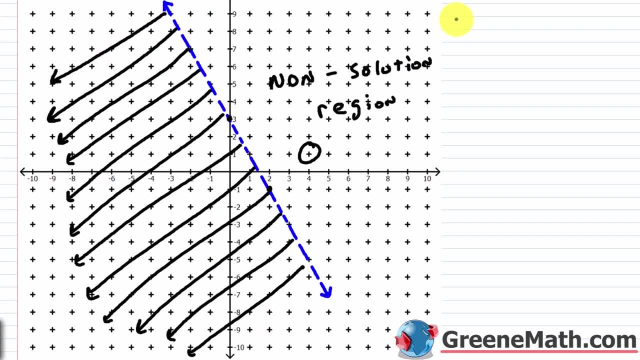 But how would I graph: y equals negative 2x plus 3? So y equals negative 2x plus 3.. Well, I have a y intercept that occurs at 0 comma 3.. So that's right here. So I would start out. 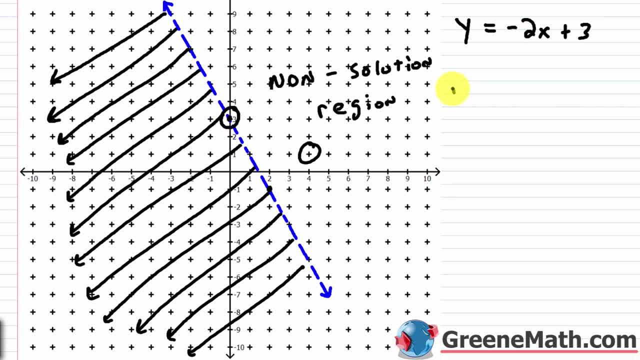 by using that point And my slope is negative 2.. So my rise over my run is negative 2 over 1.. So I would fall to 1,, 2 to the right, 1.. Fall to 1,, 2 to the right, 1.. 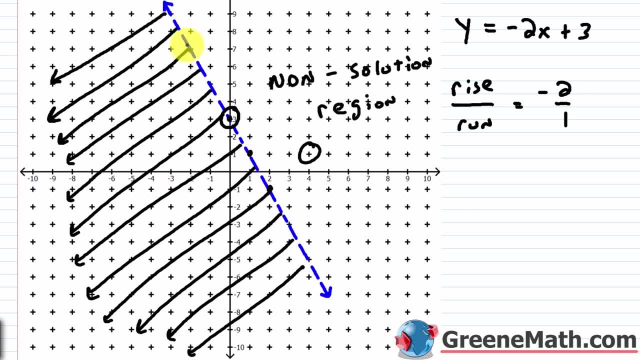 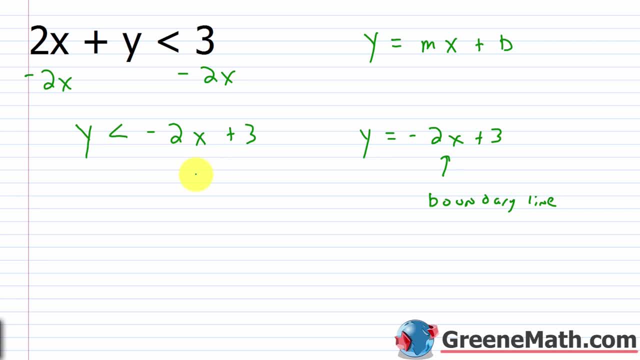 So I would draw my boundary line based on that. So I get the same exact line. Now here's where the fun part comes in. If I've solved this for y, I don't need a test point. All I do is look at. 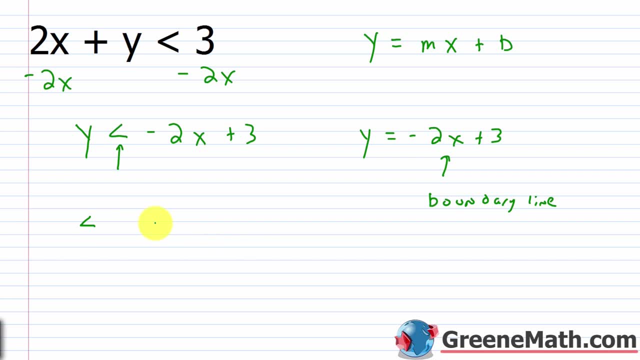 the symbol that I'm given. If I have a less than, I shade below the line, So that's a less than or a less than or equal to. Let me kind of slide that down: Less than or less than or equal to. 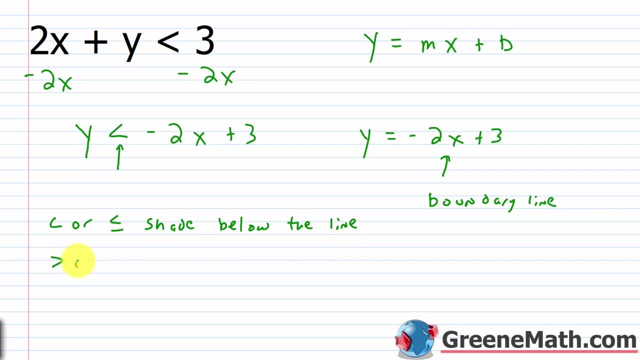 Shade below the line. If I have a greater than, or a greater than or equal to, I'm going to shade above the line. It's very, very simple. So, if I look at this, this is a less than. I just come back to the graph. 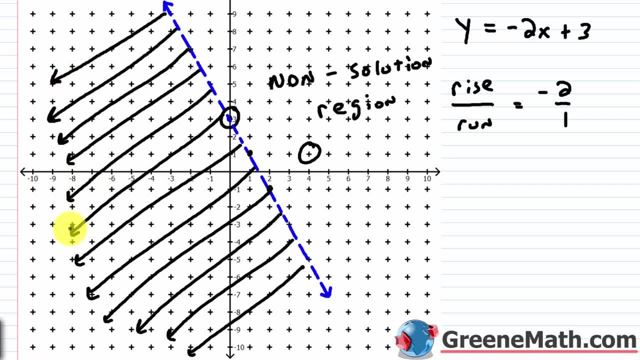 Once I have the line, I just shade below it And that's exactly what I see there. So look how much faster that would have been versus using kind of the slow method and then on top of that, finding a test point, going back to plug it in. 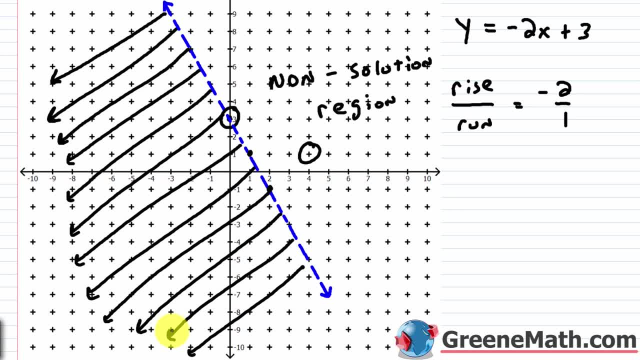 seeing if it works, then shading. So I think the test point method is quite slow actually, And solving the linear inequality in two variables for y is definitely the way you want to go. So let's take a look at another one. now. I'm going to use both methods. 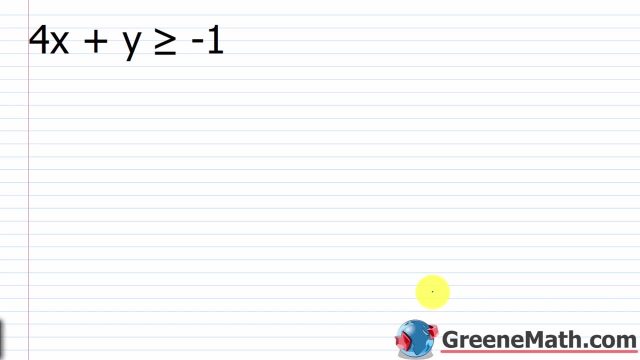 for one last time, And then, from here on out, I'm just going to solve this guy for y. I'm going to kind of blow through these. I'm going to do it by solving for y first, though, So I'm going to subtract 4x. 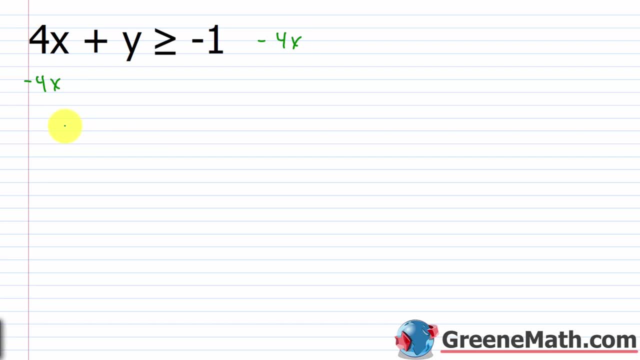 away from each side. That's going to give me: y is greater than or equal to negative 4x minus 1.. Now to get my boundary line, I just replace this with equals, So I'll have: y is equal to negative 4x minus 1.. 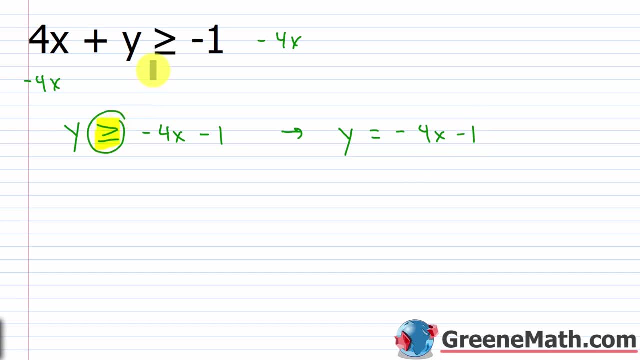 Now I want you to notice something: This is a non-strict inequality. So in this particular case, my boundary line is solid, right, Because points on that line will satisfy the inequality. So if I graph, y equals negative 4x minus 1.. 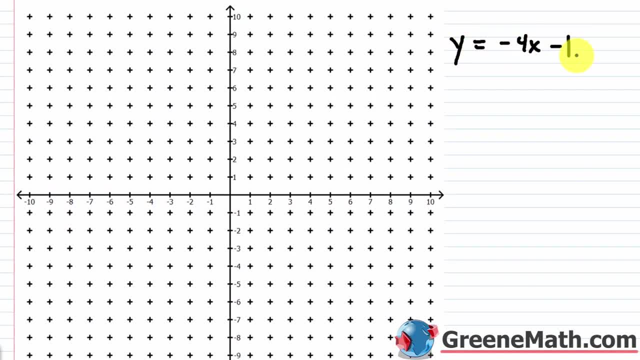 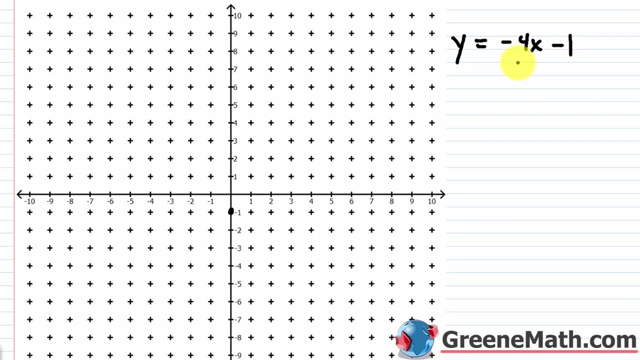 So y equals negative 4x minus 1.. My y intercept occurs at 0 comma, negative 1.. So that's right here. My slope is negative 4.. So again, rise over run: It's negative 4 over 1.. 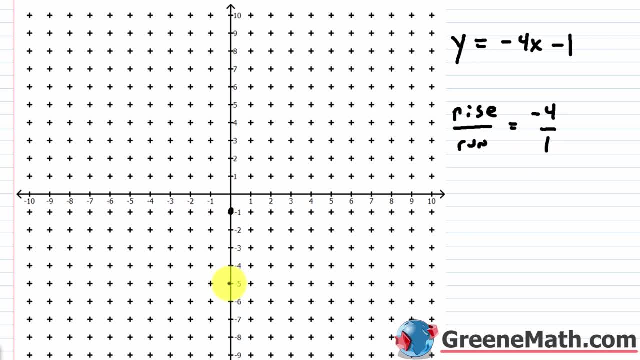 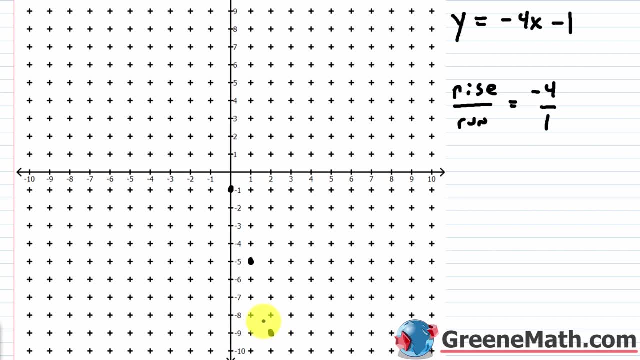 So I fall for 1,, 2,, 3,, 4.. I go to the right one. I fall for 1,, 2,, 3,, 4.. I go to the right one, Or I can think about this. 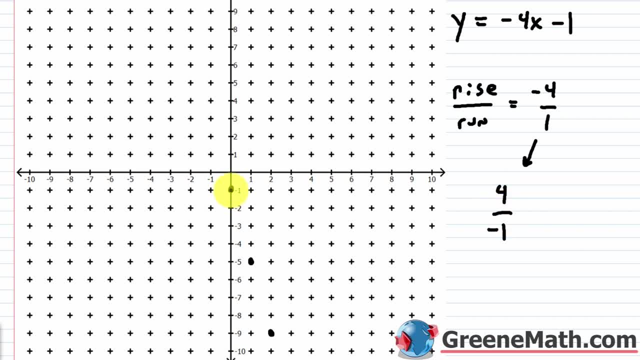 as 4 over negative 1.. So I could start here and I could go up 4.. 1,, 2,, 3,, 4.. I can go to the left one. So now, when I sketch this graph, remember this is a solid line now. 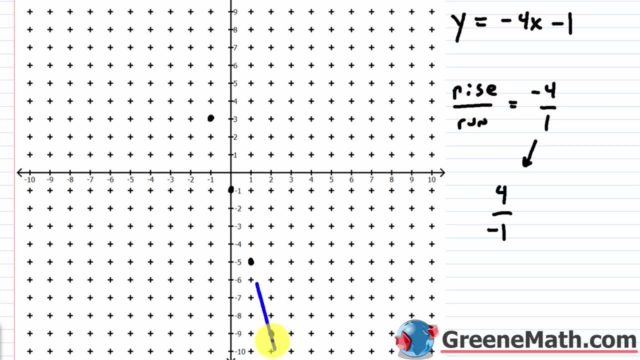 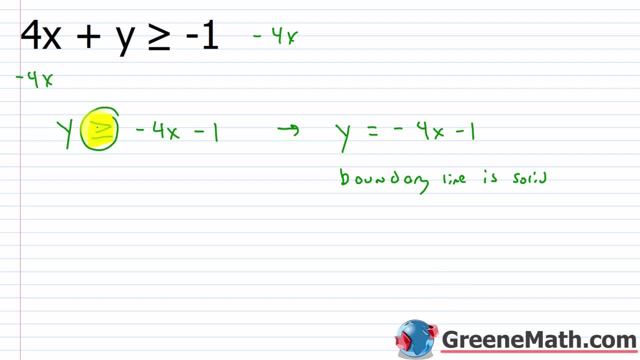 This boundary line is part of the solution, So I can use this to apply for this line Right now. the next thing I'd look at is the fact that this is a greater than or equal to. So for a greater than, or a greater than or equal to, 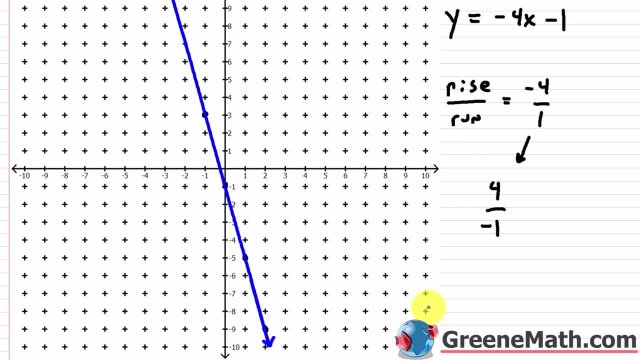 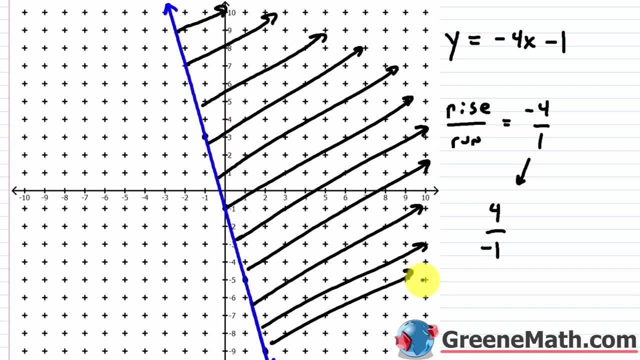 I shade above the line, So I come back here. If I want to shade above the line, I would shade this direction. Just make it completely clear to your teacher, or whoever is grading your test, that this is the solution region and then this over here. 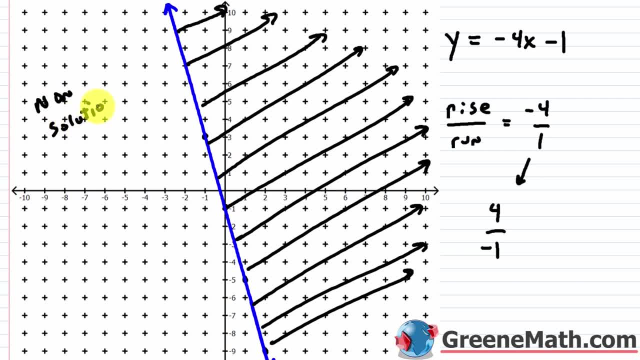 is the non-solution region region. So again, you've got three different parts here. You've got a non-solution region, where ordered pairs do not satisfy the inequality. You've got a boundary line which, in this case, will satisfy the inequality, And then you've got a solution region. Okay, so three parts here. 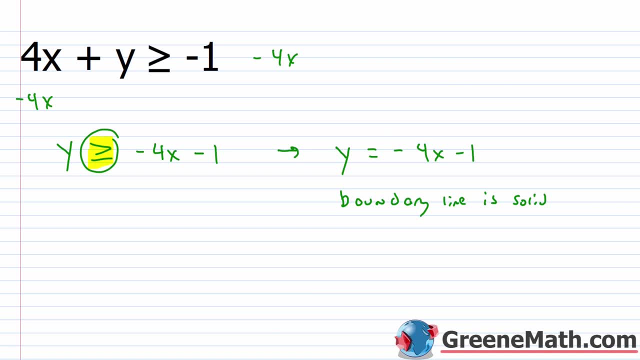 Now you saw how quickly we did that. Let's erase all of this. Let's do this the slow way, using a test point. So I'm just going to start out again by replacing this with equals. So I would have: 4x plus y is equal to negative 1.. And let's get some ordered pairs going. 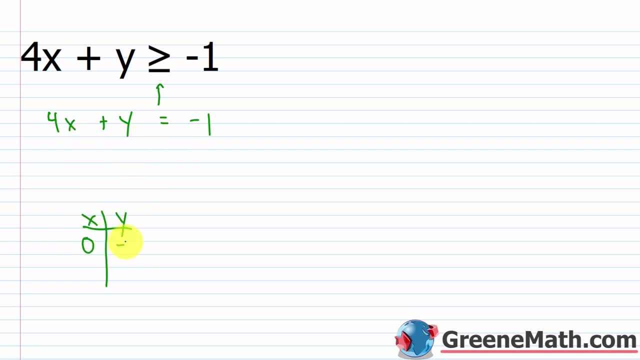 So let's say x is 0. We know y equals negative 1. Let's say that x is negative 2. We'd have 4 times negative 2 plus y equals negative 1.. 4 times negative 2 is negative 8.. 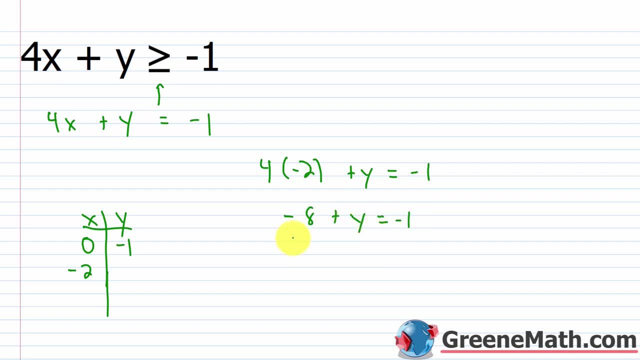 So I'd have negative. 8 plus y equals negative. 1. Add 8 to both sides of the equation. That'll cancel. You'll get y is equal to 7.. Let's try something simple for x. Let's try 1.. 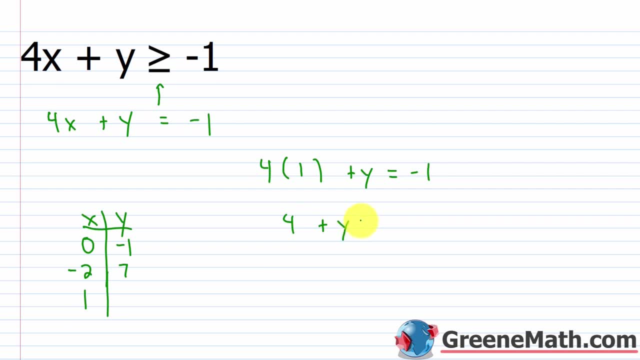 So if x is 1, 4 times 1 is 4 plus y equals negative 1.. Subtract 4 away from each side of the equation, You'll get y is equal to negative 5.. All right, so I have three ordered pairs there. 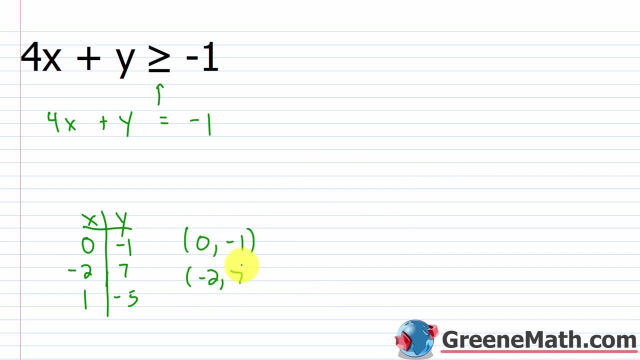 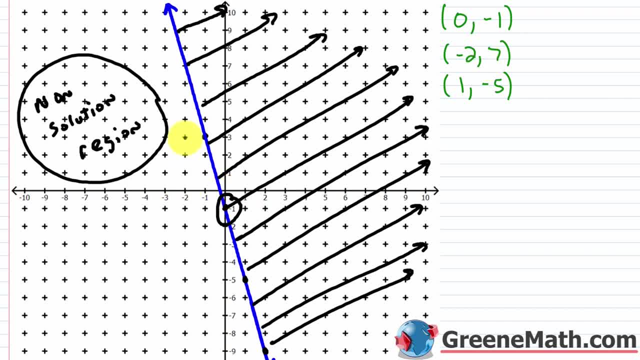 Negative: 2 comma 7,. if I go 2 units to the left and 7 units up, that's right there. And then 1 comma negative 5, if I go 1 unit to the right and 5 units down, that's right there. So my points are: 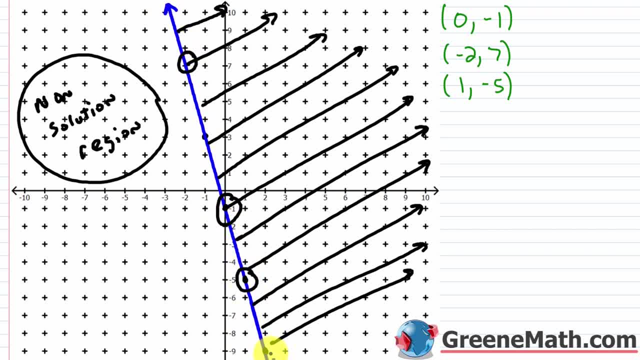 there I would draw my solid boundary line. Then I would have to choose a test point. In this particular case, I can still use 0 comma negative 1.. I can still use 0 comma negative 1.. I can still use 0 comma 0 because it's not on the line. So I would go back up here And I would say 4 times. 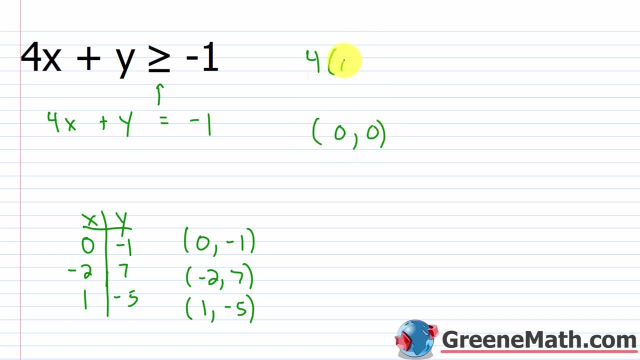 again, my test point is 0 comma 0. So 4 times 0 plus 0 is greater than or equal to negative 1.. So you'd end up with what 0 is greater than or equal to negative 1. And 0 is greater than. 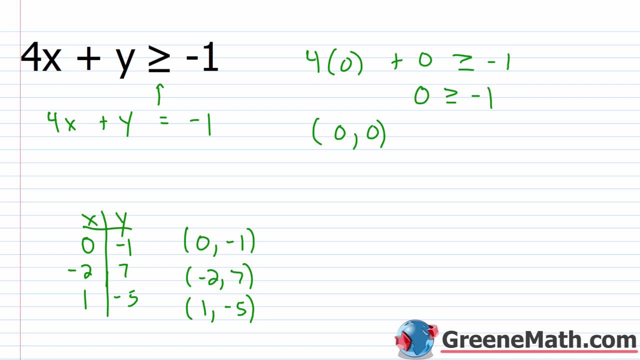 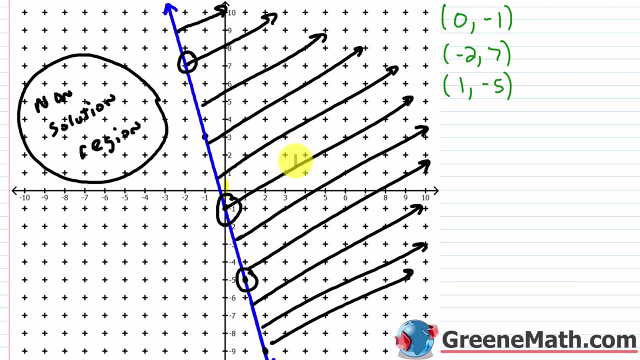 negative 1.. So that is true? So that would tell me that I need to shade above the line, And again, that's what I already found. So using a test point works. It's just a little bit slower. in my opinion, Using this method, where we solve the inequality for y, allows you to. 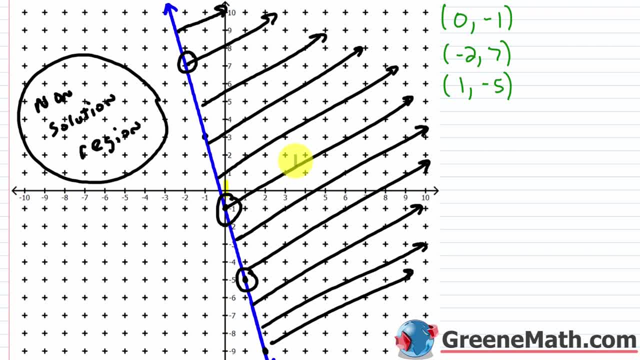 graph the boundary line faster. right, Because you can graph based on the slope and the y intercept, And it allows you to shade the line faster, because you shade based on whether it's a greater than greater than or equal to, or less than less than or equal to. Okay, So in all, 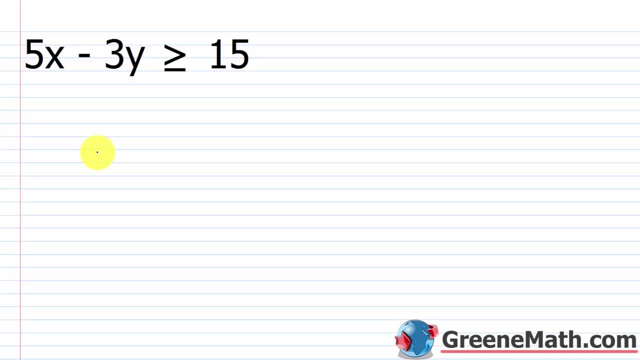 aspects. in my opinion, it's just simply faster, All right, So let's look at another one, And again, I'm not going to use a test point anymore, So let's solve this guy for y. So we have 5x minus 3y is greater than or equal to 15.. 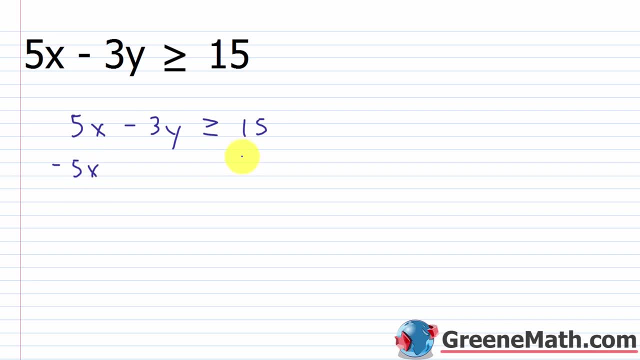 If I solve this for y, I'm just going to subtract 5x away from each side. That's canceled, I'll have negative 3y is greater than or equal to negative 5x plus 15.. Now, very important that you remember. 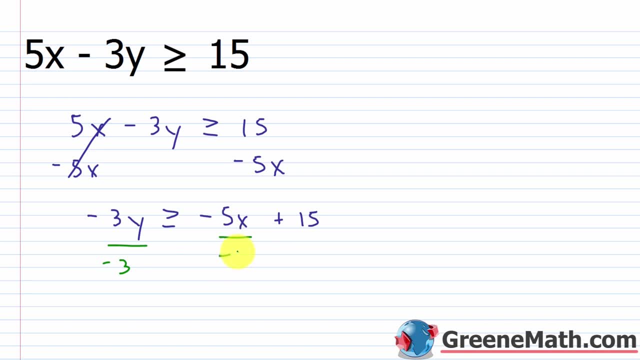 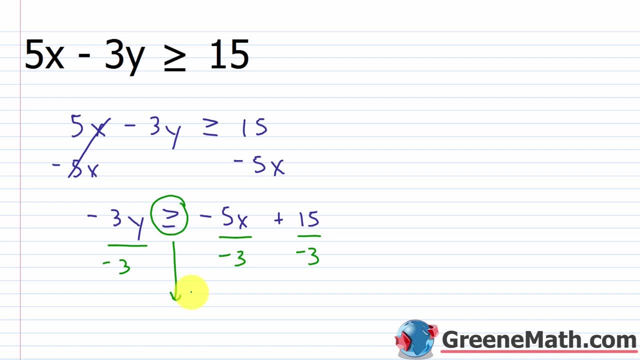 Now I'm going to just do this in the plus space of the inequality symbol. If this is 8 greater than or equal to, I've got to make sure to make this a less than or equal to. Otherwise I'm going to get the wrong answer and I'm not going to shade in the right direction. 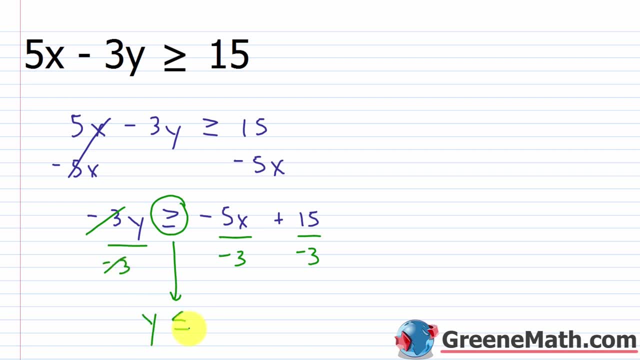 Now I'm going to just do a little bit of a flip here, So this cancels with this I've got. y is less than or equal to negative 5 over negative 3.. 1 plus 3y minus 4y. minus 4y is: 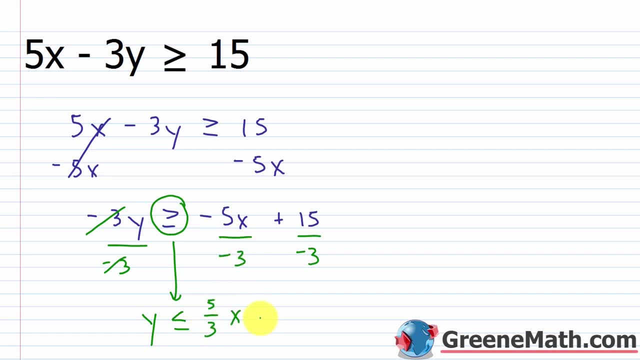 less than or equal to minus 3y, minus 4y, minus 4y, minus 4y minus 5y. So we have 5x less than or equal to minus x, And this is minus 15 over negative 3.. I have accounted for the 100 minus. 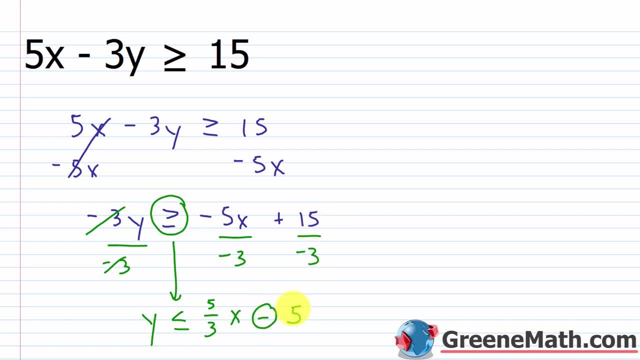 negative: 15 divided by 3 is 5, so minus 5. so I've got: y is less than or equal to 5 thirds x minus 5. so let's erase this. pull this up here and again. I still want to graph my boundary line, so I'm just. 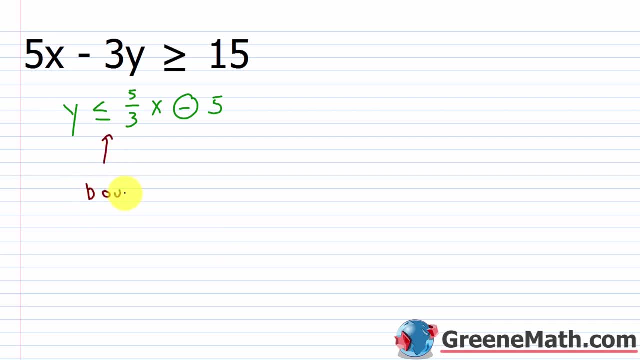 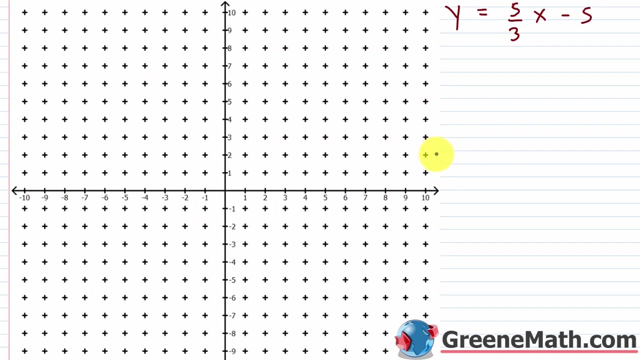 going to replace this with equals. so my boundary line I would have y equals 5 thirds x minus 5. now again, because this is a less than or equal to, it's a non-strict inequality. so that tells me that points on the boundary line will satisfy the inequality, and so I want a solid line, all right, so? 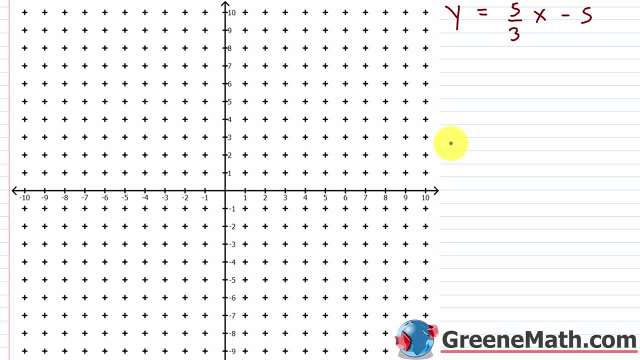 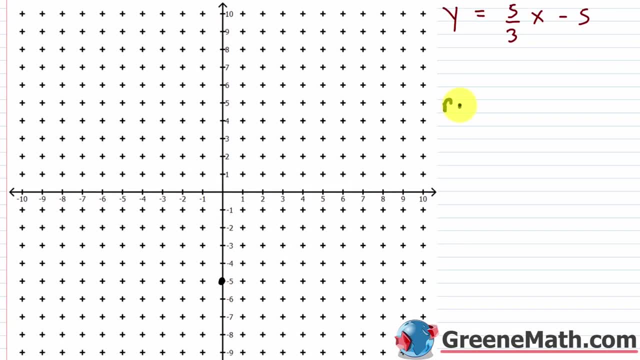 the graph, y equals 5 thirds x minus 5. I know the y intercept here is at 0 comma negative 5. it's right here. my slope is 5 thirds, so my rise over my run is 5 over 3. so I'll: one, two, three, four, five to the right. one, two, three, then again up. one, two, three, four, five to the right. 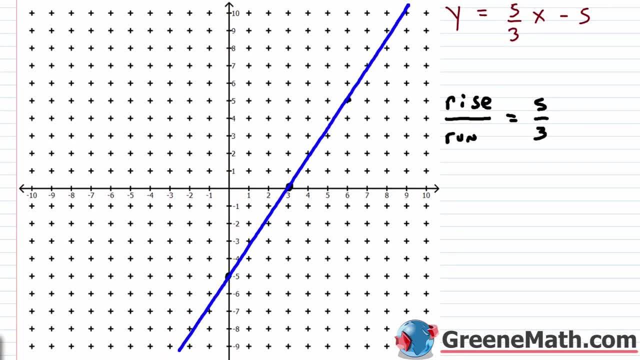 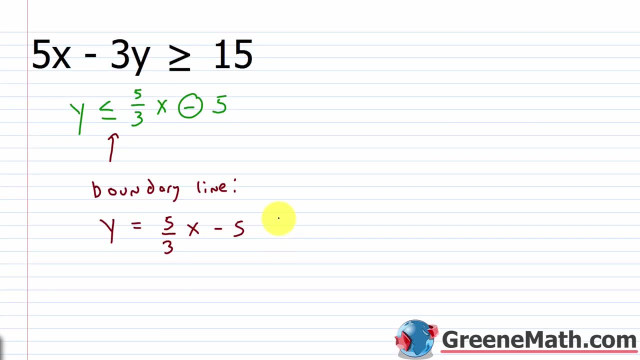 one, two, three, and let me erase a little part of that. it's a little little long for us, so put arrows at each end. so this is my boundary line. again, it's a solid line because we have a non-strict inequality. now, if I go back to my page, I see that when I solved it for y, I have a less than or equal. 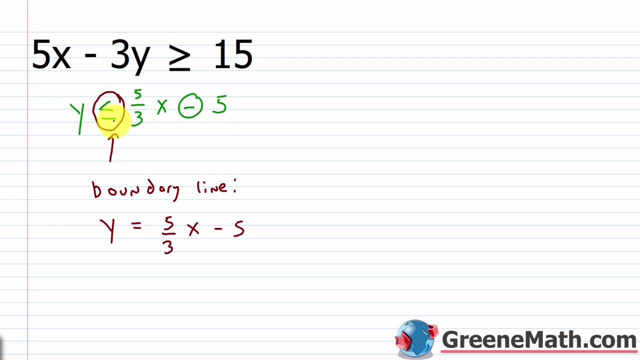 to. so that means I'm going to shape it up and I'm going to shade below the line. again, it's got to be solved for y. you don't want to look at this original guy. make sure it's solved for y first. y is less than or equal to, so that means I shade below the line. 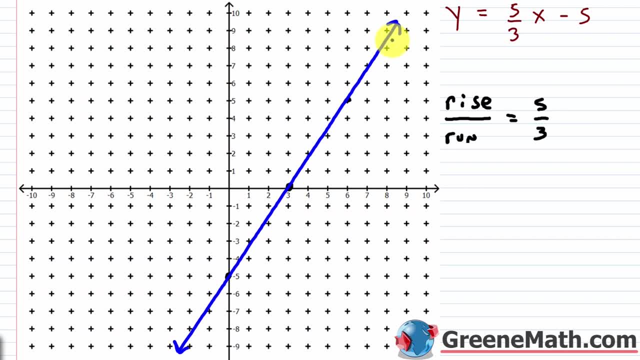 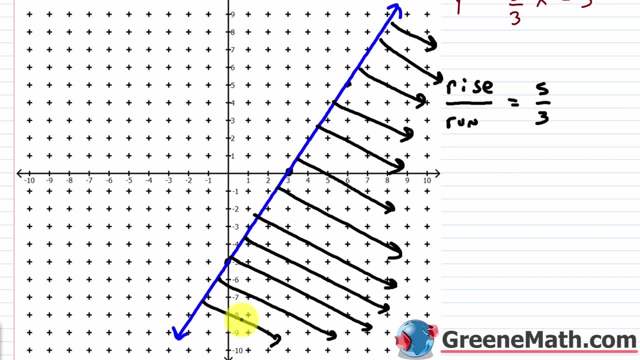 so if I look, if I want to shade below the line, I would shade this way. so anything shaded that's in the solution region, the boundary line, is part of the solution here and then anything over here above that line is in the non-solution region. so these points will not work. 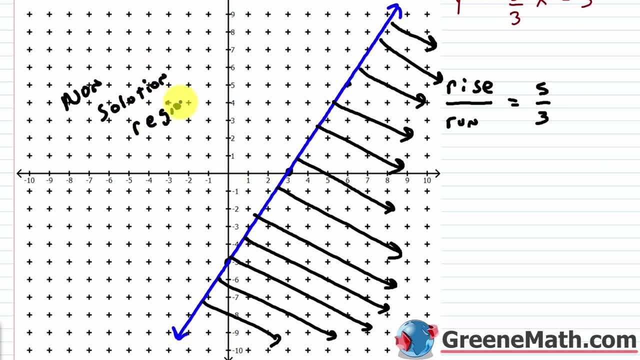 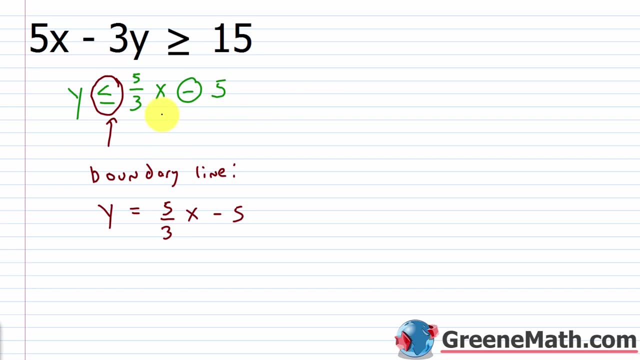 and you can always grab a test point to check. you can take zero comma, zero notice. that's in the non-solution region. so if we plug it in it should not work. so if I go back up here I can take and plug it into this one or the original, doesn't matter. 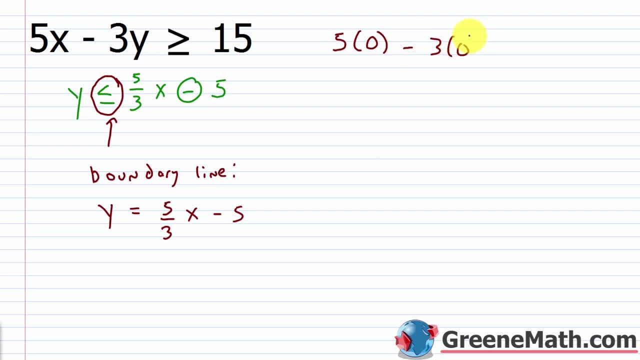 so five times zero minus three times zero should be greater than or equal to zero, and then I can go back and plug the value into zero, and then I can go back and plug it into the original again. this should not work, so we expect this to be false. this will cancel. this will cancel. you'll get zero. 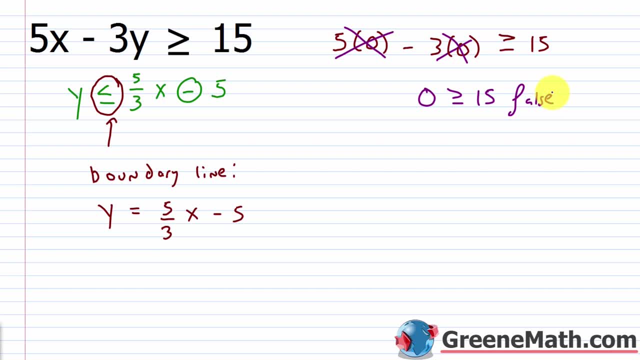 is greater than or equal to 15, which is false. zero is not greater than 15 and zero is also not equal to 15. but again, that's what we expect, because 0 comma 0 is in the non-solution region. all right, so let's talk about some special case scenarios now. let's say you came across: y is greater than. 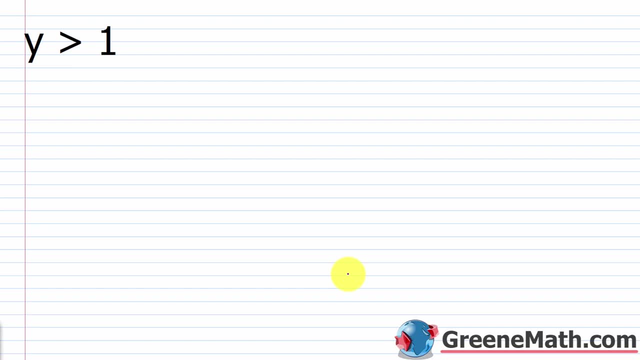 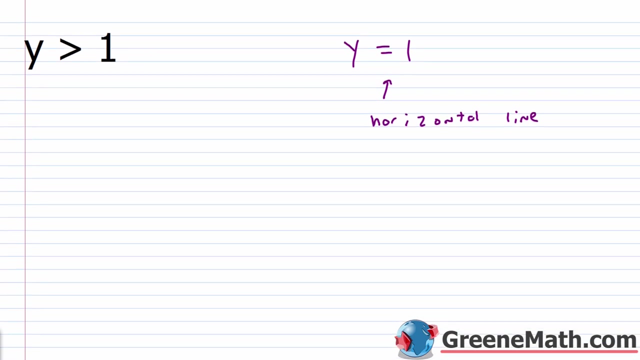 1 and you're like: what do I do there? y is greater than one. remember a few things here. For one, if you had, y equals 1, this is a horizontal line. This is a horizontal line. So to graph this I would go to my coordinate plane. And again I'm thinking about: 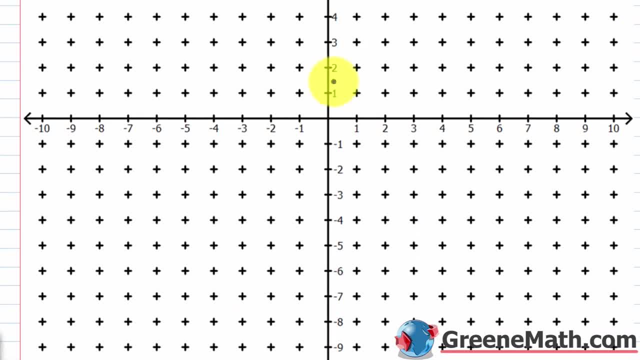 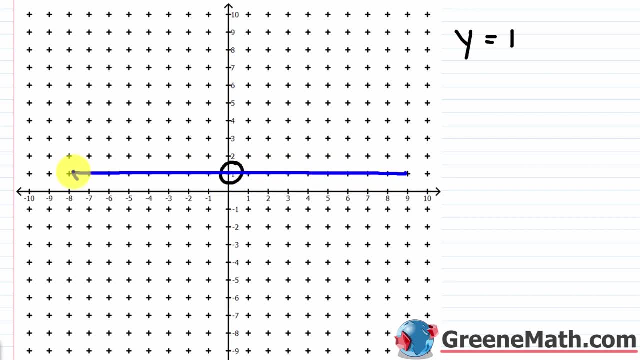 y equals 1.. So find 1 on the y-axis. It's right here. I would just draw a horizontal line. So this would be y equals 1.. When we look at this, we see that this is a non-strict inequality. 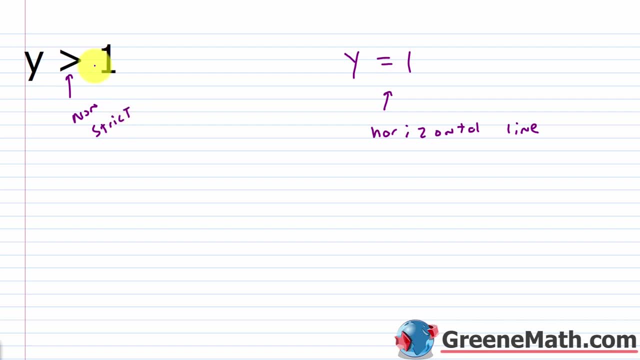 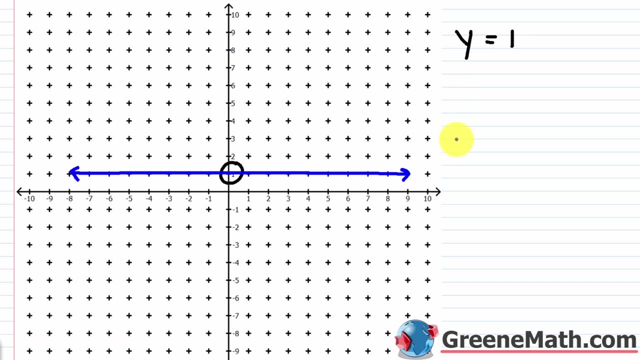 This is non-strict, So we know that points on the line will not satisfy that inequality. So what we do is we make this a dashed line. So y is greater than 1. We would have a dashed line- Let me take my eraser now- and we will break this guy up. And again, this identifies that. 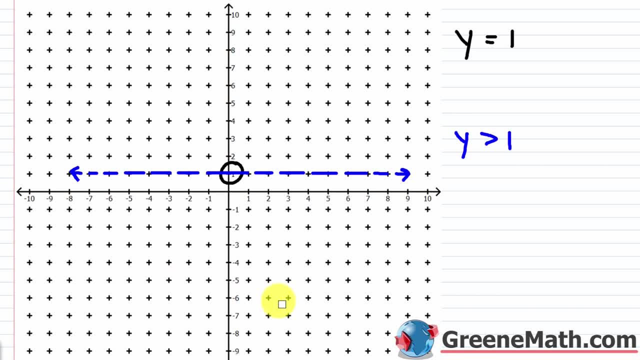 points in this line are not part of the solution. Now, if y is greater than 1, what does that mean in terms of a solution? Well, that means anywhere on the y-axis that's larger than 1 is a solution. So that means I would shade above the line. 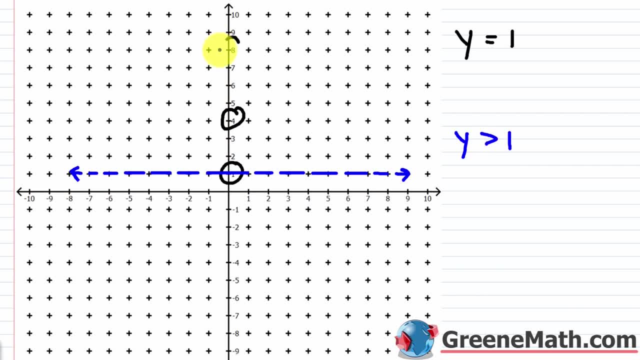 because if y is 4,, 4 is greater than 1.. If y is 8,, 8 is greater than 1.. Anything below the line doesn't work. If y is negative 1,, well, that's not greater than 1.. So that wouldn't work. So this down here would be the non-solution region. 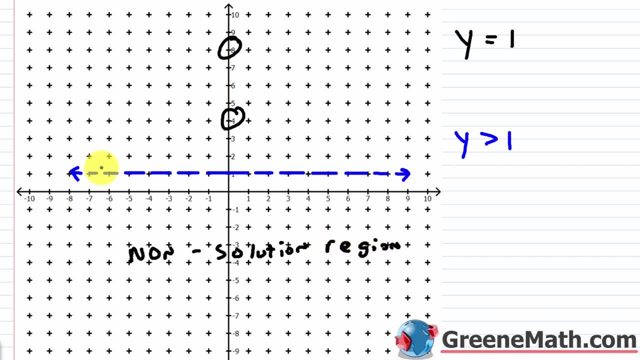 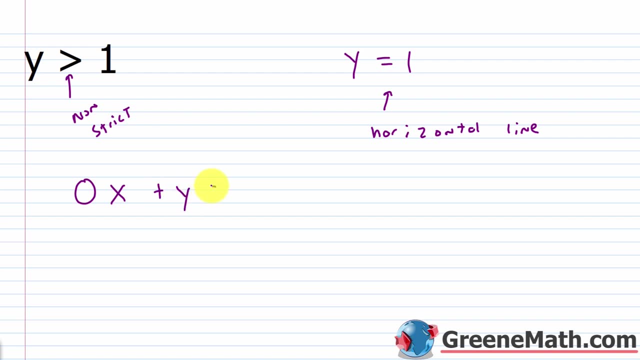 and anything above the line would be the solution region. So I would shade this way And again: how do you check something like that? Well, formally again, if you think about something like 0x plus y is greater than 1, well, if I choose a point, 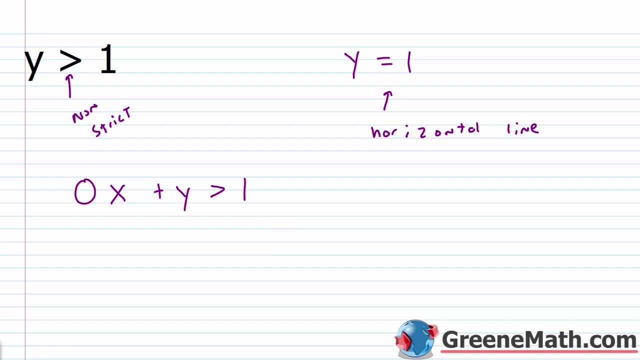 where y is greater than 1, I'm going to be able to say that y is greater than 1.. Well, if I choose a point where y is greater than 1,? well, if I choose a point where y is greater than 1,, it's going to work out. So, if I choose a y of like, let's 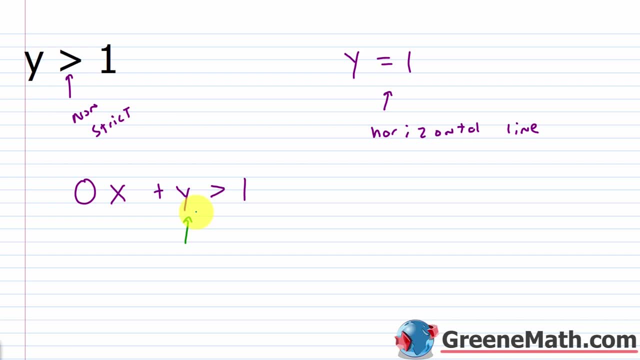 say 5, for example, x can be whatever, x can be negative 30. So let's say I have a point: negative 30, comma 5.. Plug in a negative 30 there. Plug in a 5 here. Negative 30 times. 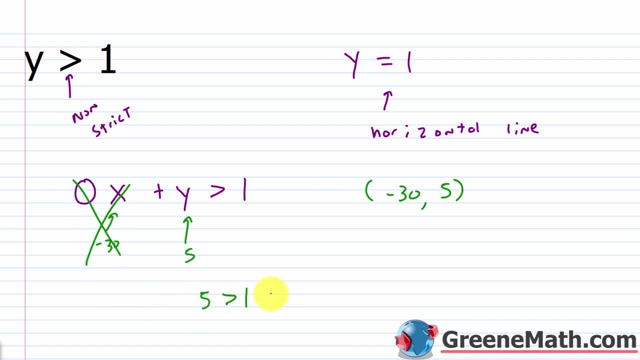 0 is 0. So that's cancelled. You'll get: 5 is greater than 1, which is true. So it doesn't matter what the value of x is, It's irrelevant As long as the y value is larger than. 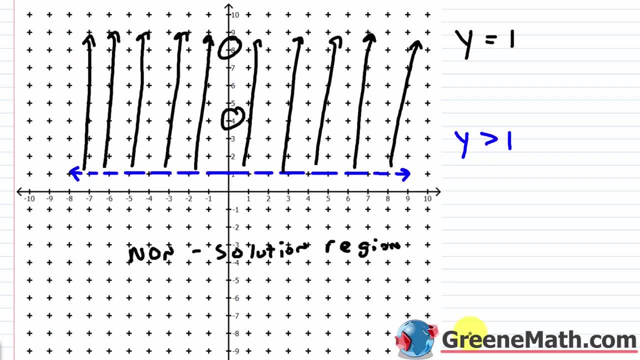 1, we have a true statement, which is y. on our coordinate plane we just shaded everything above the line. Again, you're just looking at y values. So you're only looking at the y axis in this case, And anything on the y axis that's larger than 1 going up is going. 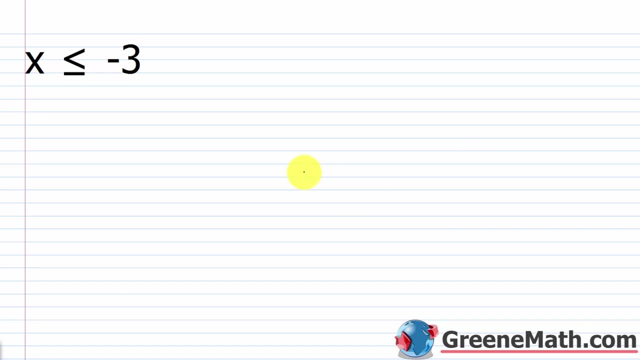 to work as a solution, All right. So, as the other special case scenario, let's say you saw something like: x is less than or equal to negative 3. So you can almost guess what this is right If I graph x is. 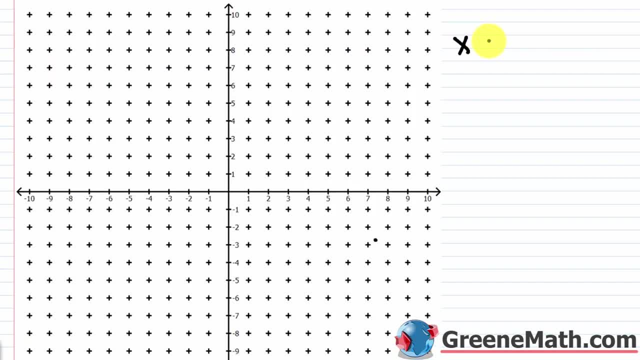 equal to negative 3, what does that look like? So x is equal to negative 3.. I find negative 3 on the x axis and I draw a vertical line. Now in this particular case we have: x is less than or equal to negative 3.. So the boundary 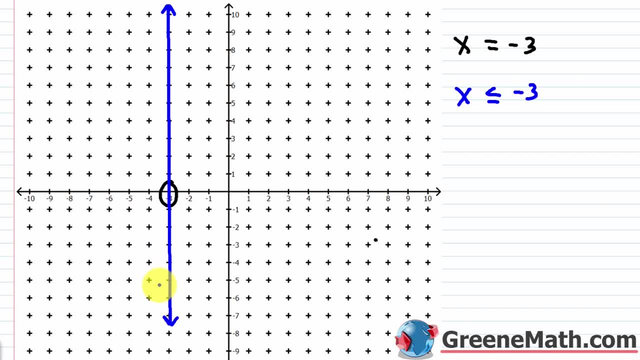 line is a solid line, So I don't need to break this up, because points on that line will satisfy the inequality. If I have x, that is actually negative 3, negative 3 is less than or equal to negative 3.. That's true. 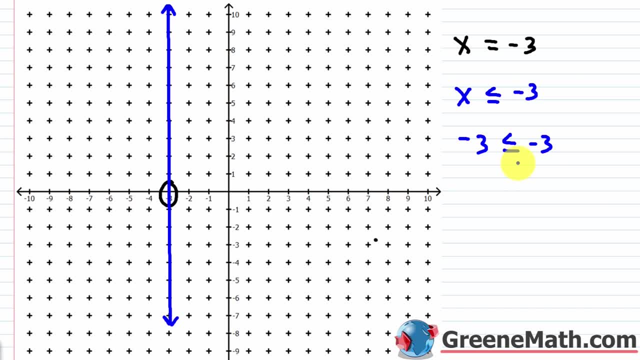 If I have x that is indirectly less than or equal to negative 3, negative 3 will be less than or equal to negative 3.. Then also, any x value that is less than negative 3 will work. So how do we get less when we're talking about the x axis? Well, we go to the left. 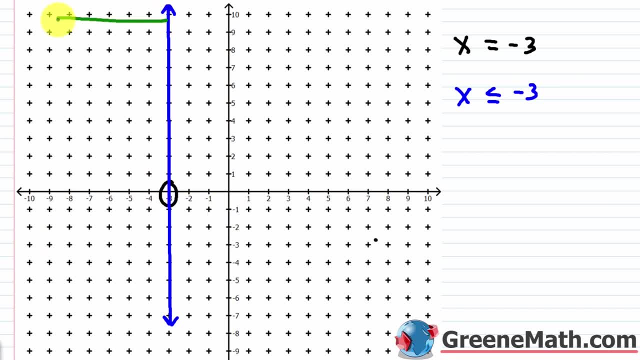 So, thinking about x values that are less than negative 3, I would shade to the left. I would shade to the left. You just have to think about this in terms of x values only, Because it doesn't matter what the y value is. 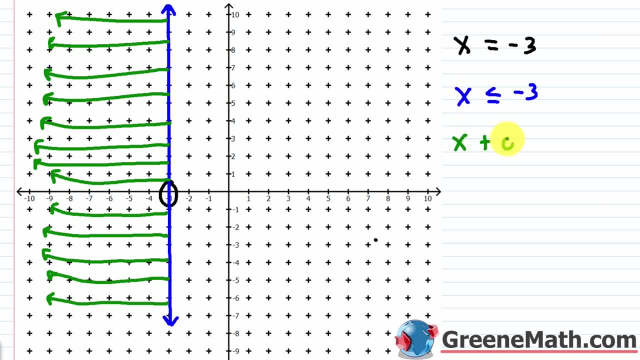 Y value can be whatever. If I wrote this as x plus 3.. So I would choose y And then I would say: x is less than or equal to negative 3, negative 0, y is less than or equal to negative 3,. you could choose a y value as high or low. 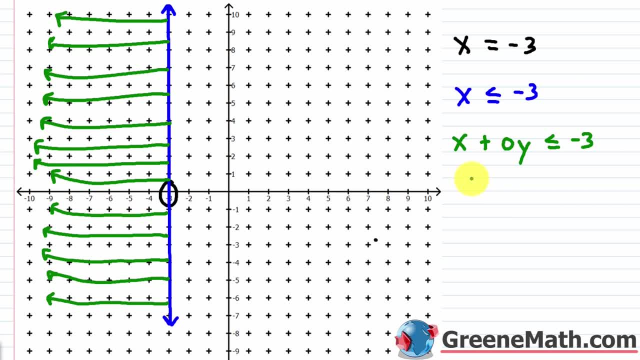 as you want. Let's say you choose 10, for example. So if I choose an x value- that's, let's say, negative 6, and a y value of 10,, this is going to work because my x value is less than negative 3.. 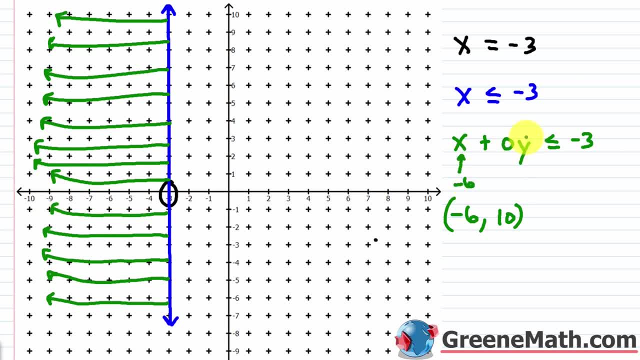 Plug in a negative 6 there. This would cancel whatever. it is 0 times anything is 0. So negative 6 would be less than negative 3, so that would work out. If you choose any x value that is greater than negative 3, it won't work out. 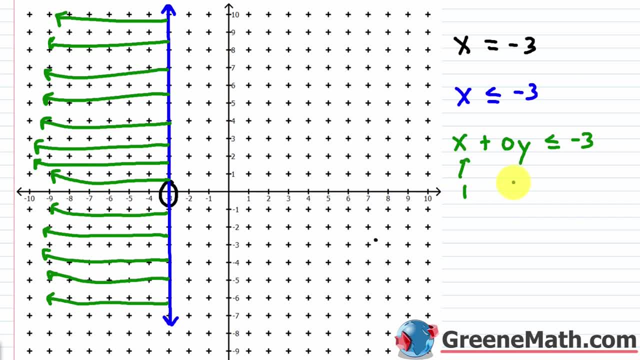 In other words, if I plug in a 1 here and let's say I use 10 here, well, 1, 10 won't work, because again this cancels One is not less than negative 3, and it's certainly not equal to negative 3,, so that 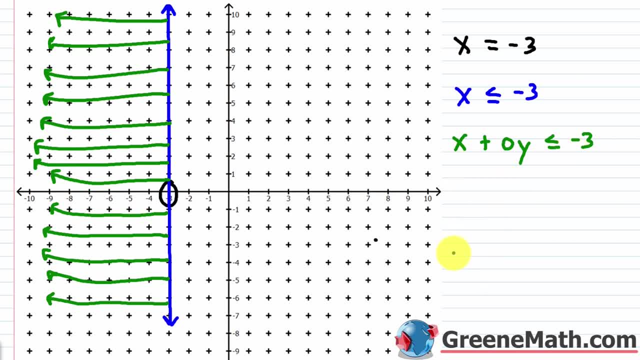 won't work. So again, when you're shading here, just think about that. Any x value that's less than negative 3 or equal to negative 3 would work. So you've got a solid line at negative 3.. And you've got values to the left of negative 3 all shaded. 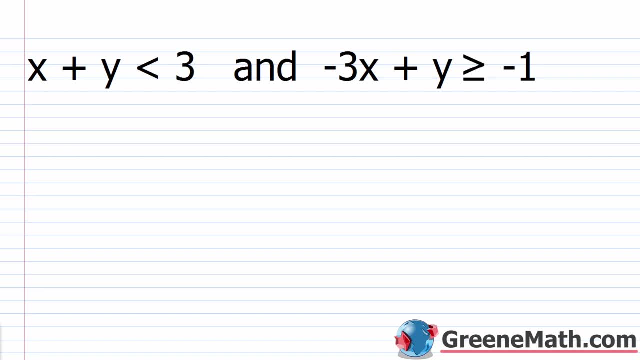 OK, so we're just going to wrap up the lesson now by talking about compound inequalities again. So we looked at these when we talked about linear inequalities in one variable. You will see them when you talk about linear inequalities in two variables, But again, this stuff is not more complicated. 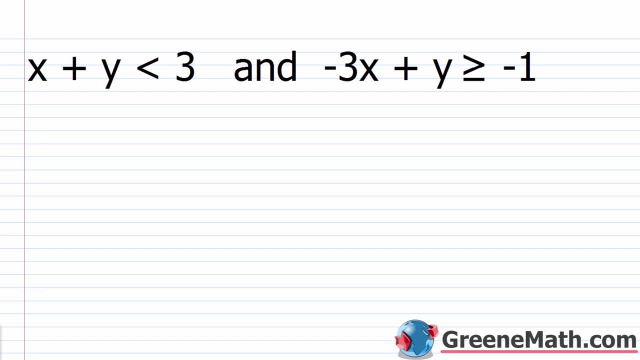 It's a little bit more tedious because we've thrown another variable in there, But graphing this should not be mentally challenging for you. Let's talk about the two different words that you're going to come across. You have AND, and then you also have OR. 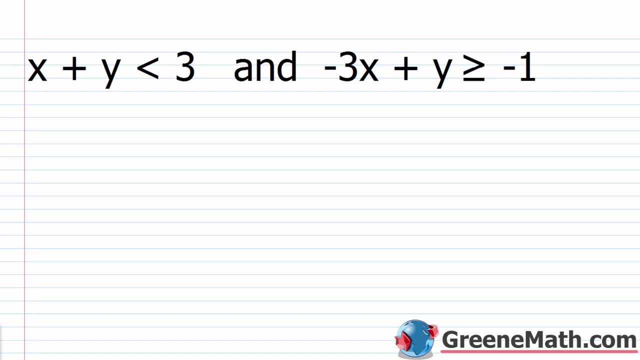 When you see a compound inequality with, AND remember you're looking for the intersection of the two solution sets. So in order to say it's a solution for the compound inequality, it has to be a solution for both. So graphically, I'm looking for the section of the coordinate plane that's the overlap. 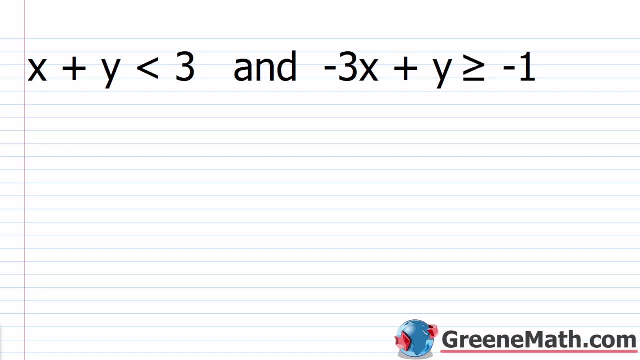 right, It satisfies both inequalities. If I'm thinking about OR right, The keyword OR. well, in that case it could be a solution to either right, So it could be a solution to one and not the other, or it could be a solution for both. 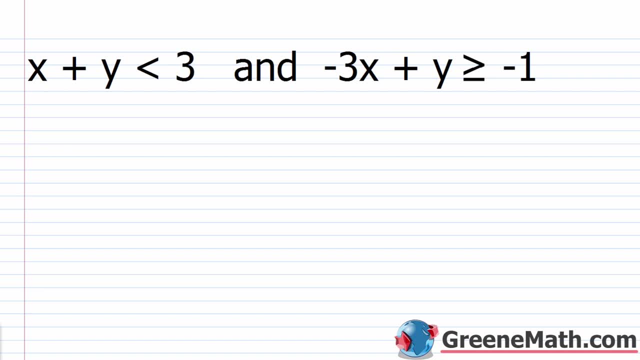 It doesn't matter because it could work for either, All right. So let's just look at this one problem here. When we go into our practice set, when we go into our test problems, we'll see a scenario with OR. Here we're just going to see a scenario with AND. 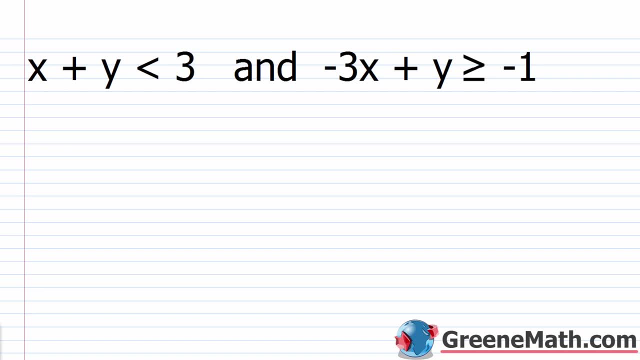 But again, if we looked at OR, we'd know the difference is it could be a solution for either. So we look at: x plus y is less than 3, and negative 3x plus y is greater than or equal to negative 1.. 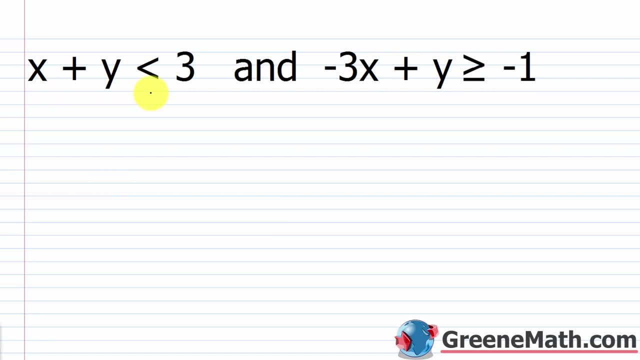 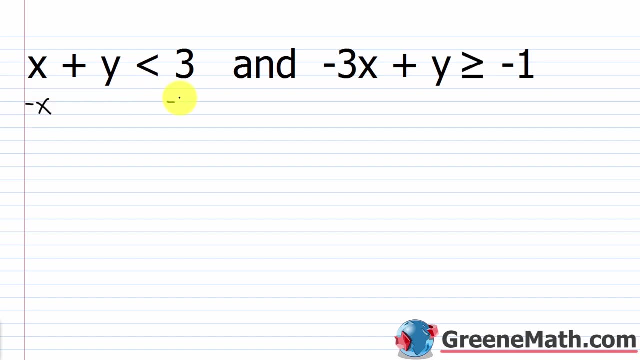 So again, I'm just going to start out by solving each for y. I'm going to graph each and then I'm going to look for the overlap. So let's start out by subtracting x away from each side over here. So that's going to give us: y is less than negative x plus 3.. 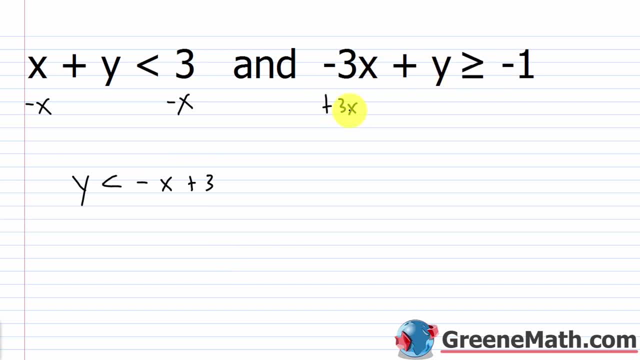 And then for this guy over here, I'm going to add 3x to each side. So that's going to give us y is greater than or equal to 3x minus 1.. So let's go ahead and take these two down to the coordinate plane. 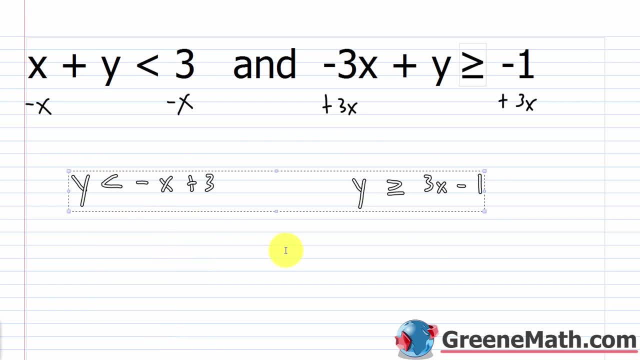 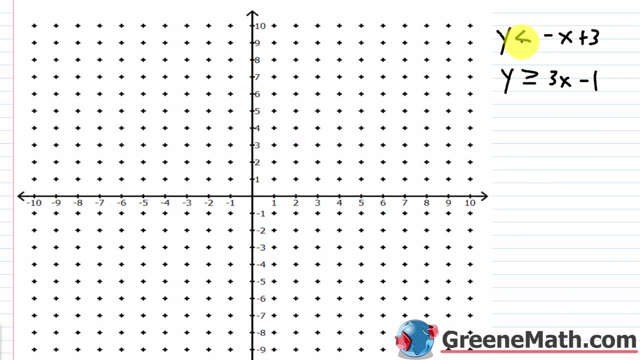 We'll just copy them And we're going to graph each one separately And then we're going to look for the overlap of the two graphs. So for the first one, y is less than negative x plus 3.. Again, to draw the boundary line, I would replace this with equals. 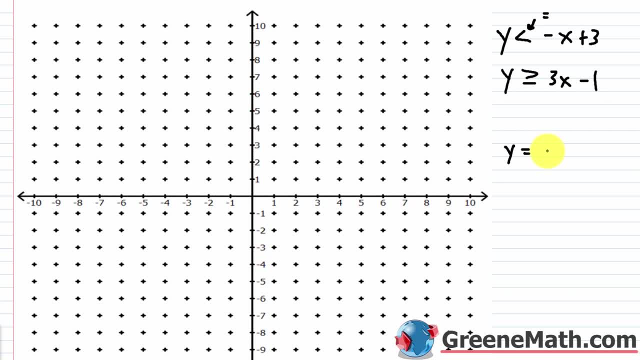 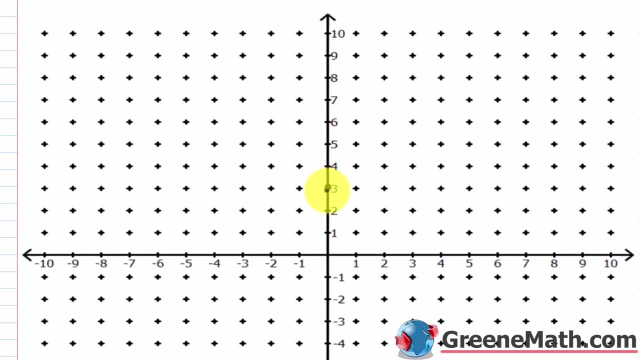 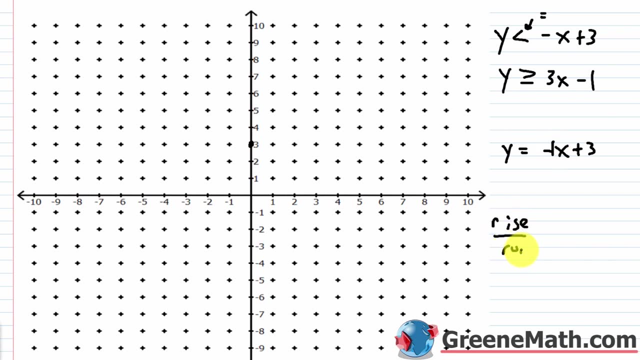 So if I had y equals negative x plus 3, how would I graph that? Well, the y-intercept is at 0 comma 3.. So that's going to be right here, And then the slope is negative 1.. So that's rise over, run of what. 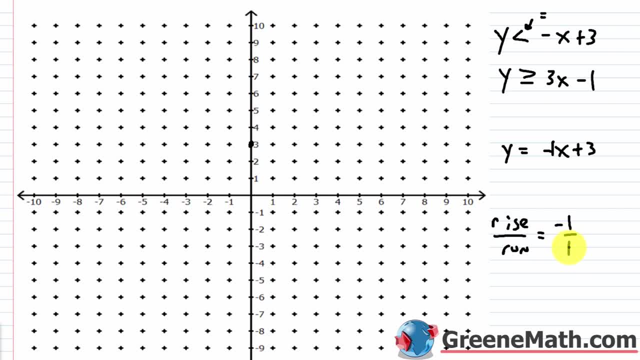 Negative 1 over 1, or 1 over negative 1, whichever you want to do. So I can fall- 1, go to the right, 1.. Or I could rise- 1, go to the left- 1, whatever you want to do. 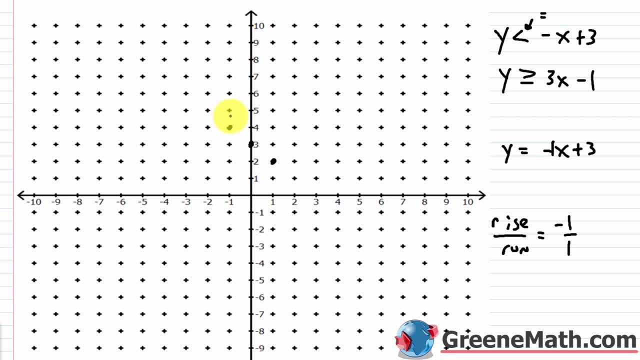 Again, if I have enough points to draw a straight line, then I'm good to go. In this case you have a negative 1.. So I could say negative 6 over 6 if I wanted to. So I could fall 6, 1,, 2,, 3,, 4,, 5, 6, go to the right: 1,, 2,, 3,, 4,, 5,, 6.. 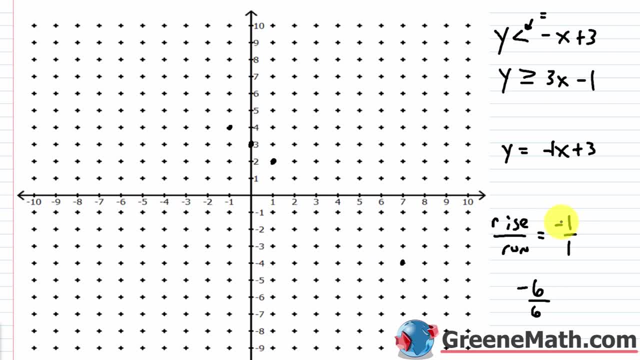 That's a point on that line, because negative 6 over 6 is negative 1.. I could also rise 6 and go to the left 6 if I wanted to, But the reason I did that was to get a point down here. 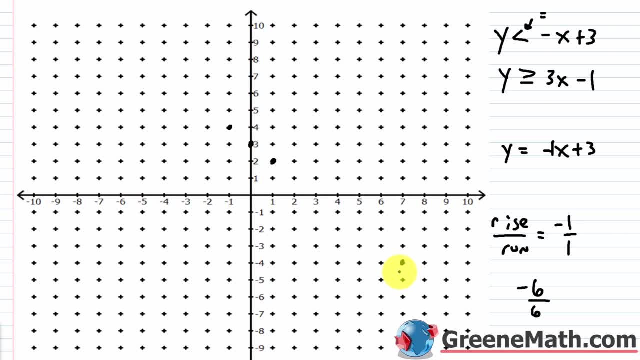 So I could kind of Put my ruler in a row and get a nice clean line. You only need two points to make a line, but it's just so much easier if you have more points involved so you can make a nice clean line. 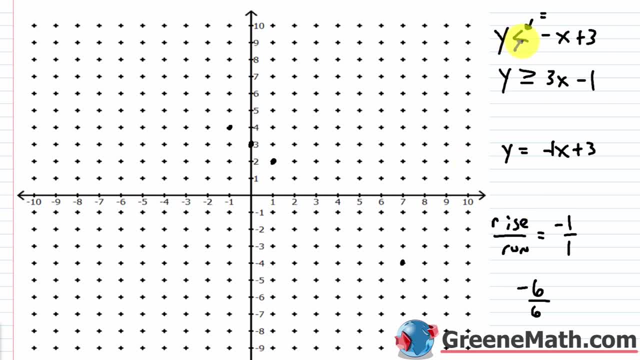 So now that I'm going to draw this- remember, this is a strict inequality, So I want a broken or dashed line, So I'll draw my line to start, put some arrows there, And what I want to do is just take my eraser now and I'm just going to break it up to 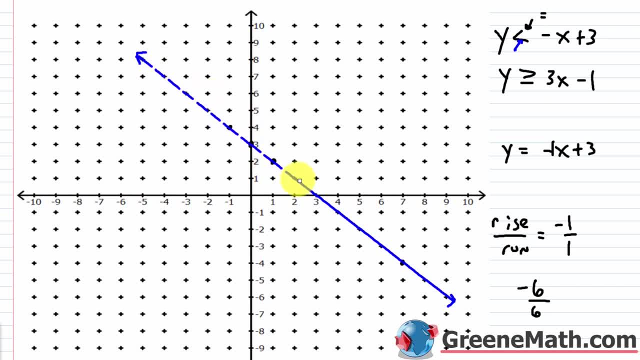 let people know if they're looking at this. this line is not part of the solution. Anytime you see a dashed or broken line, you know it's not part of the solution. All right, Now we have a less than So. if we have a less than, we're going to shade below the line. 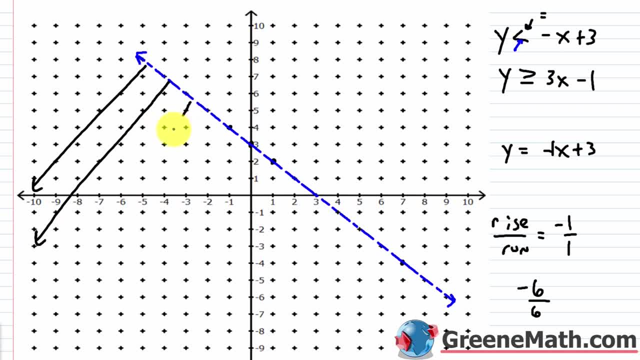 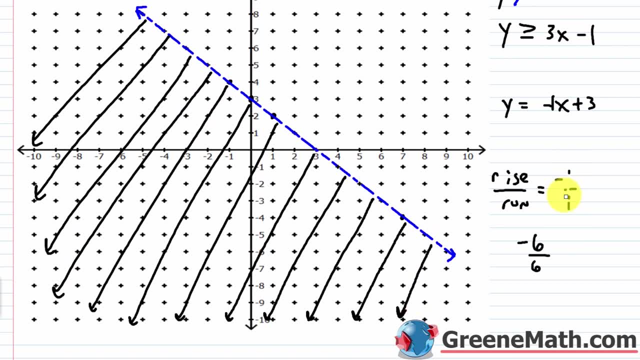 So I want to shade below the line like that. Let's look at This: is greater than, or equal to, 3x minus 1.. In this case, I'm just going to erase this And I'm just going to change this to a stroke eraser. 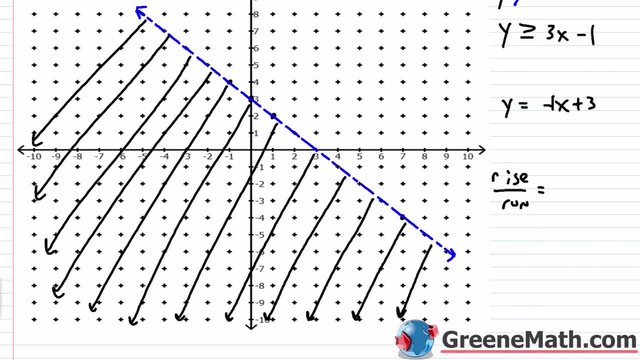 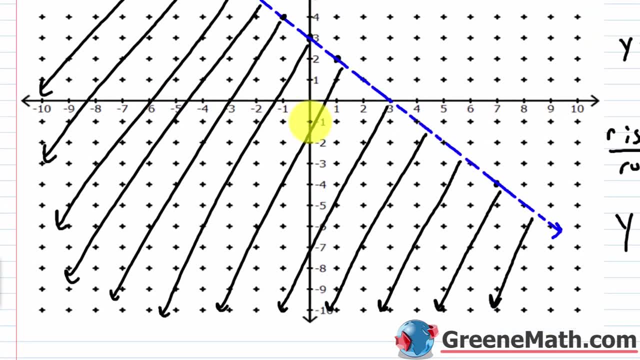 I can erase quickly. In this case I have y is equal to 3x minus 1 for my boundary, So I'd go to 0 comma negative 1, which is here, And my slope is 3.. So rise is 3 over run, which is 1.. 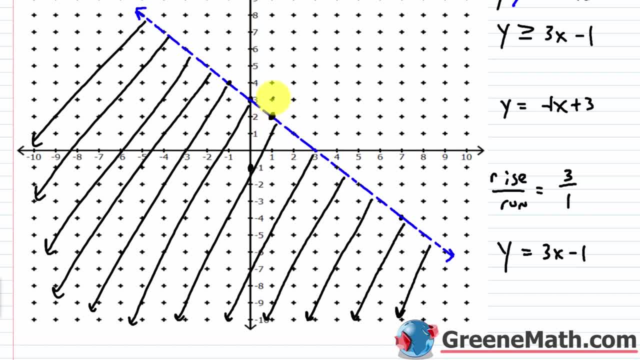 So up 1,, 2,, 3, go to the right 1.. Up 1,, 2,, 3, go to the right, 1.. Or I could fall: 1,, 2,, 3, go to the left. 1, because 3 over 1. 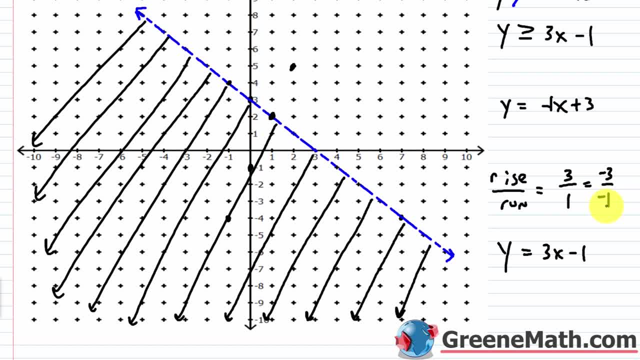 is equal to negative 3 over negative 1.. Again, think about those tricks. So I'm going to draw this line in green And this line right here is going to be a solid line, because this is a non-strict inequality. 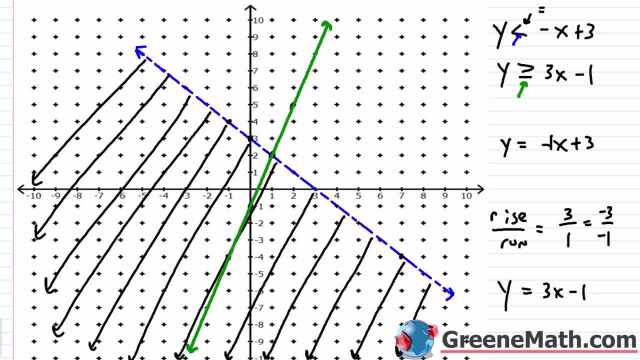 So this is a greater than or equal to, So I want to shade above the line, So I'm going to do that in an orange. OK, so this is a non-strict inequality. So what I'm going to do is I'm going to use a black marker on my line here. 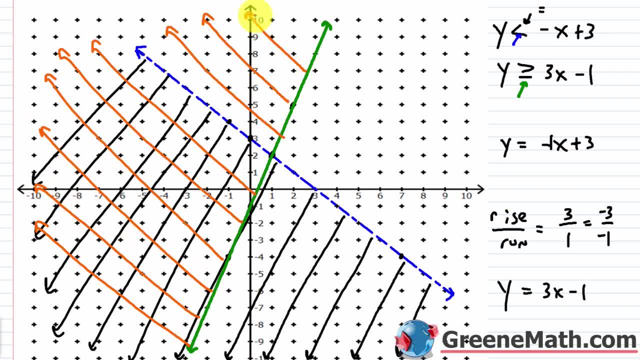 I'm going to do the x plus 2. And I'm going to do a value of 0.. If I'm looking for the overlap, the section on the coordinate plane that satisfies both- the thing that I want to do, the thing that makes it easier for me- I'll take a black marker. 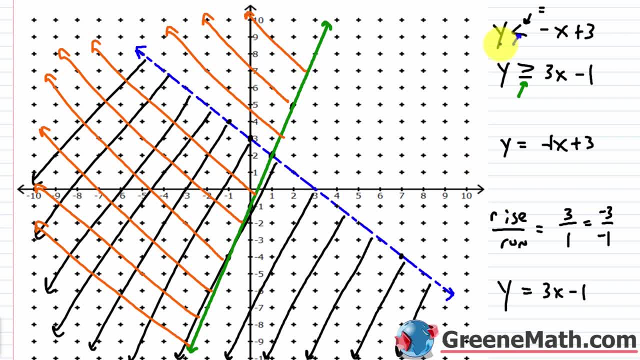 And I'll start lining out stuff that does not work. So in the first case, y is less than negative x plus 3.. We know we had this blue dashed line. Any point that was below that line worked as a solution. So any point above the line doesn't work as a solution for this inequality and therefore 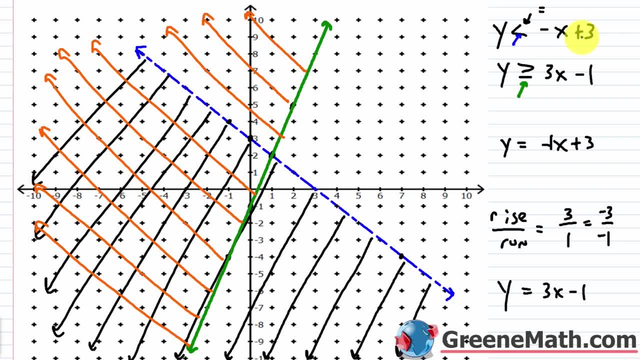 doesn't work as a solution for the compound inequality, because it has to work for both. So I can just take a little black marker or whatever a pencil and just mark this section out and say, hey, this is not going to be part of the solution for the compound inequality. 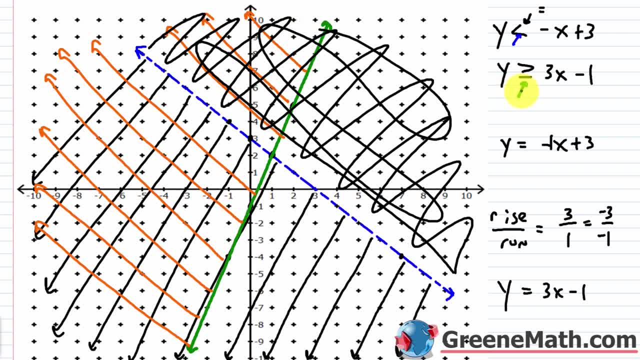 Then I'd look at the next part. Y is a greater than or equal to 3x minus 1.. OK, well, that was this green line here. So anything above the line worked. Anything below the line didn't. So this is where it's below the line. 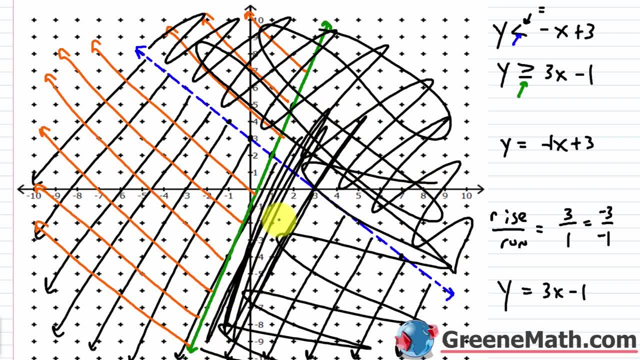 And that does not work. Now, what's interesting here is that the green line in this case is actually part of the solution. With the blue line, it's not right. It's the difference between a strict inequality and a non-strict inequality. 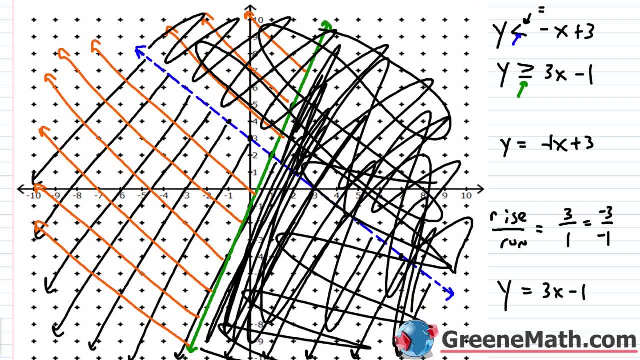 But when I look at the overlap, I'm just going to highlight this with a normal highlighter. now The green line here, starting at this intersection point, is included. So I would highlight all the way down here And at some point I have to stop. 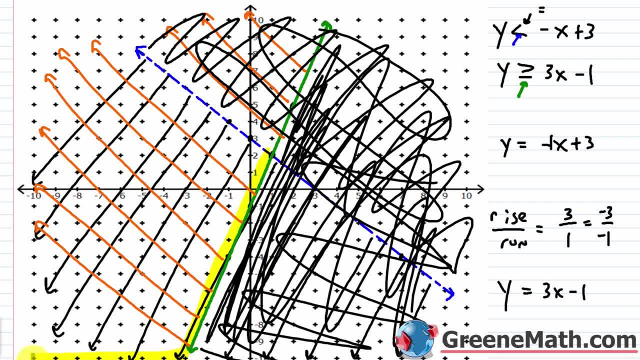 But this is an infinite area And all the way over here And all the way up here And then all the way here, And then this blue line here is not included. So I'm just going to highlight that. So the green line that's highlighted here, that's included. 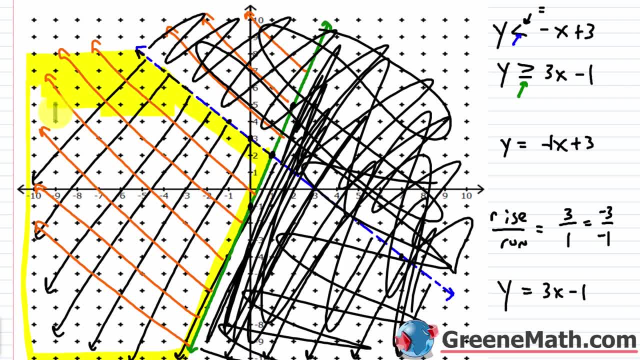 The blue line not included, And then I'm just going to shade everything here in this area. This is the section of overlap, or the part of the coordinate plane that satisfies both inequalities, And so this is the solution for the compound inequality with and. 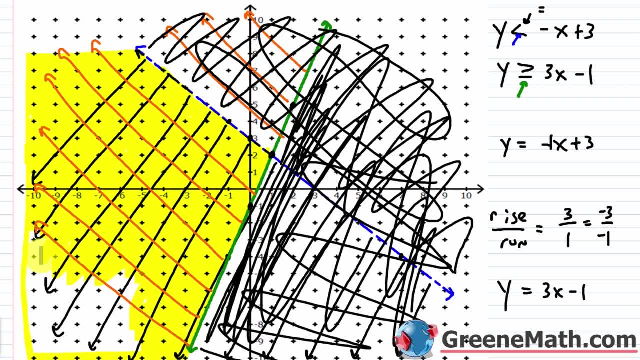 Now, if you had had a compound inequality with or, again, you would be highlighting the sections that satisfied either right, It wouldn't matter if it satisfied both, It would be what satisfied either one. But for our problem here we had and. 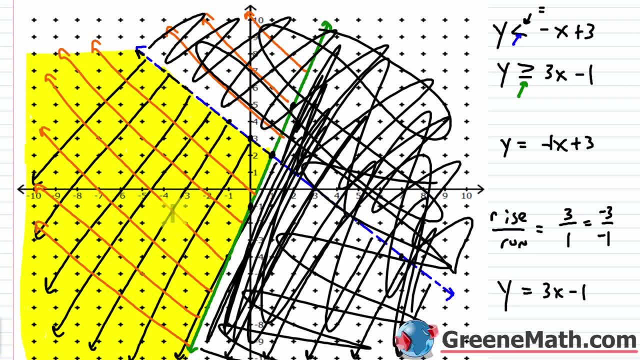 So this is a good representation. Of course, you can always make it better If you wanted to. If you wanted to get a little bit better, we could erase this arrow here And we could kind of extend this line a little more. 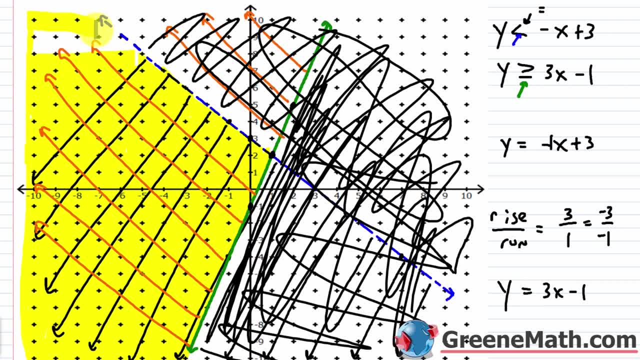 And let me give a highlighter again. I'll just kind of highlight a little bit more here, Just get a better representation, a better visual aid here. But you're basically saying to your teacher: hey, anything that's above the green line. 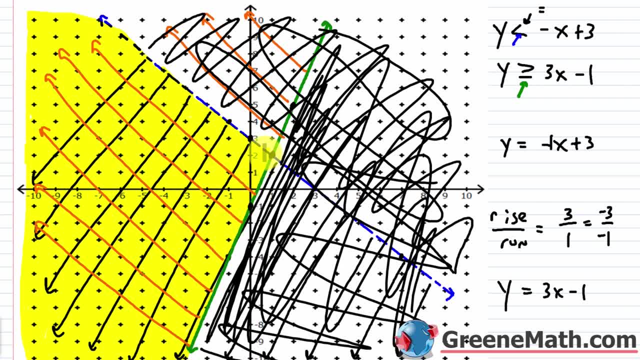 right, starting right here, going to that intersection point And including And including that green line that is also below the blue line, not including the blue line, is the part of the coordinate plane that satisfies both, And so that's your solution for the compound inequality, in this case with and. 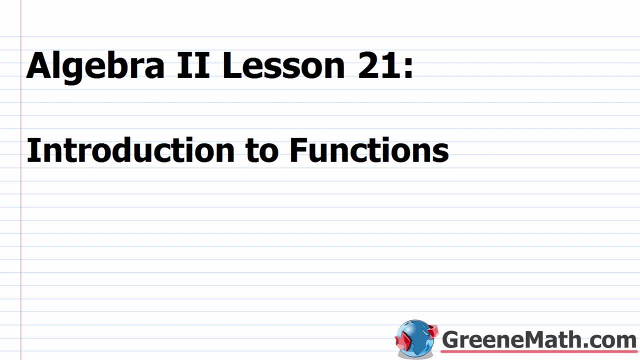 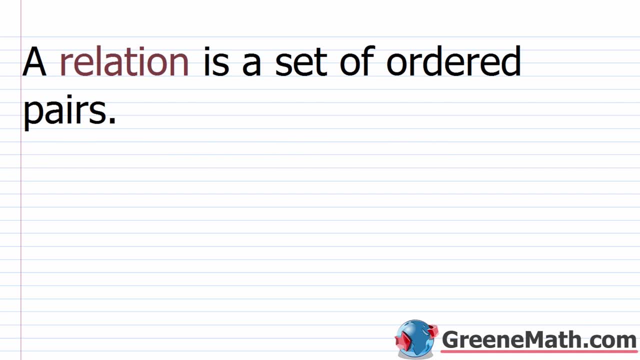 Hello and welcome to Algebra 2, Lesson 21.. In this video we're going to have an introduction to functions. So if you took an Algebra 1 course, you at least got a basic introduction to the topic of functions. In this Algebra 2 course we're going to go a little bit further than we did in Algebra. 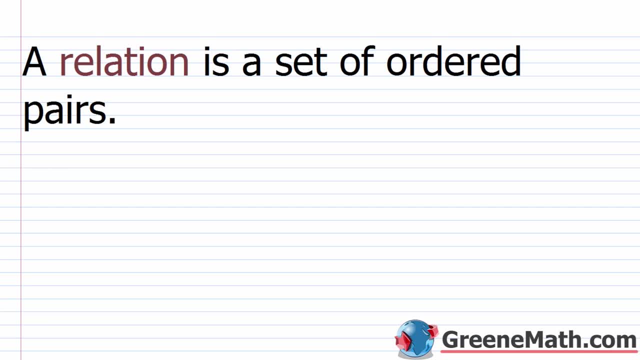 1. We're going to start today with a brief introduction And then over the next few lessons, we're going to look at some more challenging material that relates to functions. So if we're going to talk about functions, we've got to start off by talking about relations. 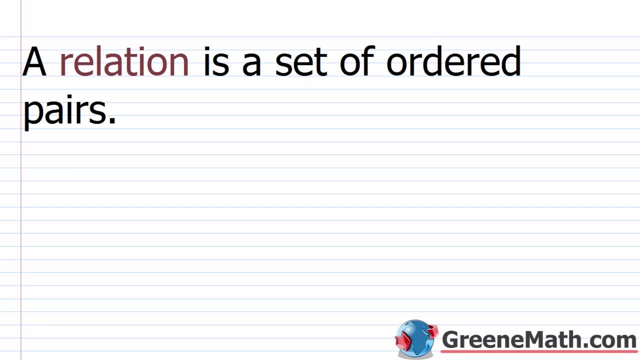 Those of you who know about functions know that all functions are relations, but not all relations are functions, And we'll get to that later. Starting out talking about relations, It is useful in mathematics- Mathematics- to be able to describe one quantity as it relates to another. 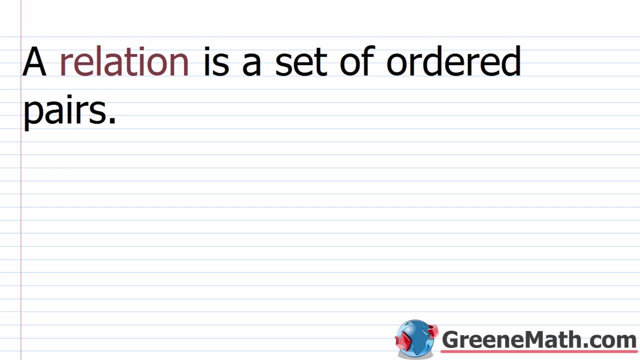 So we talk about this concept of a relation. So a relation is just a set of ordered pairs And we talk about a set again. that's a collection of some stuff. So to get a little bit of an understanding here, let's look at an easy example. 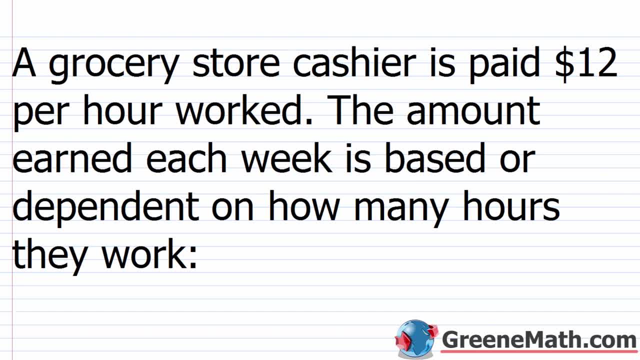 Let's say that you're given this scenario. So we have that a grocery store cashier is paid $12 per hour worked, So $12. Per hour worked. The amount earned each week is based or dependent on how many hours they work. How many hours they work. 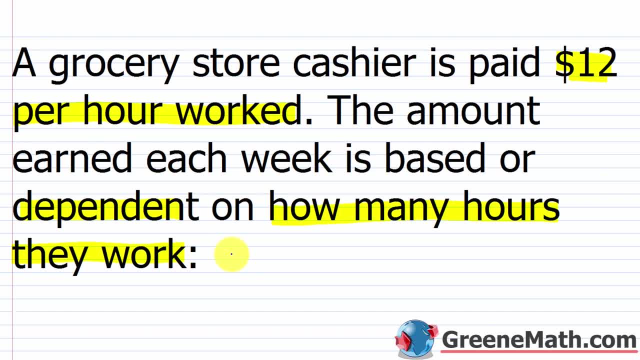 So for anybody that works hourly, you know that you take the amount you make per hour and multiply it by the number of hours you work And that gives you the amount of your gross paycheck. When I say gross paycheck, I mean the amount before any deductions. you know taxes anything. 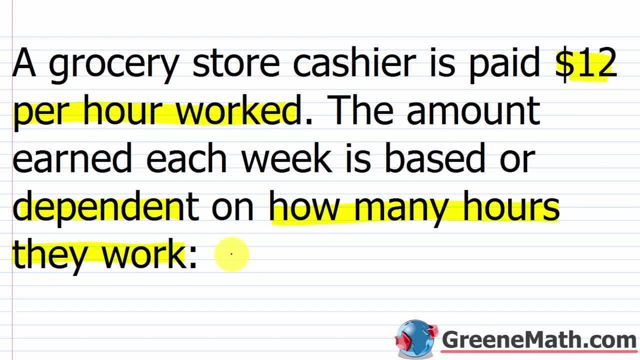 you have removed from your paycheck. So to model this we can use two variables. I would let one variable, let's say X, be equal to the number of hours worked. So if I multiplied $12, which is the amount earned in an hour, times the number of hours, 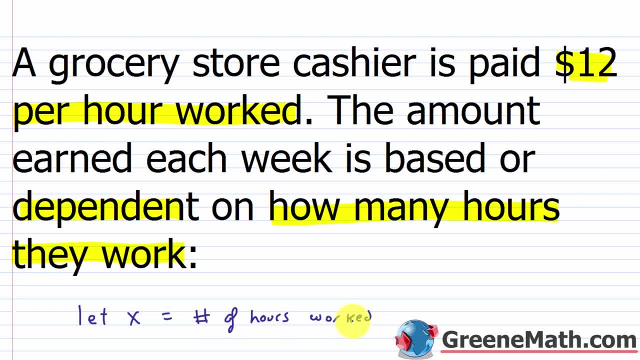 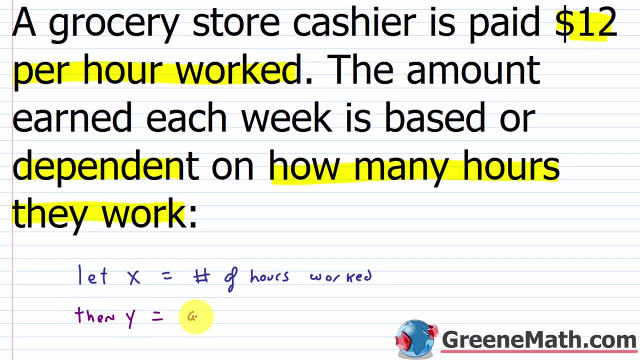 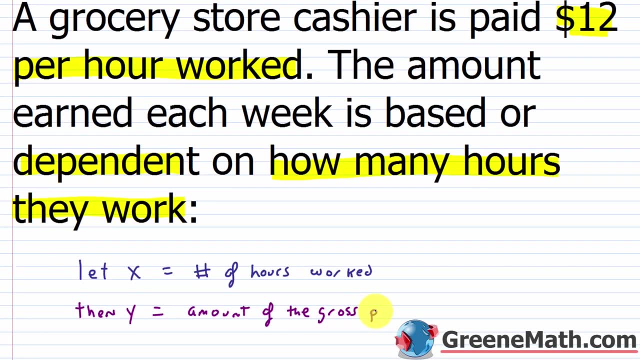 worked, I would get a gross paycheck. So let's let something like Y. Let's say then Y Would be equal to the amount of the gross paycheck. So I can take 12, again the amount earned per one hour. multiply it by X, which represents: 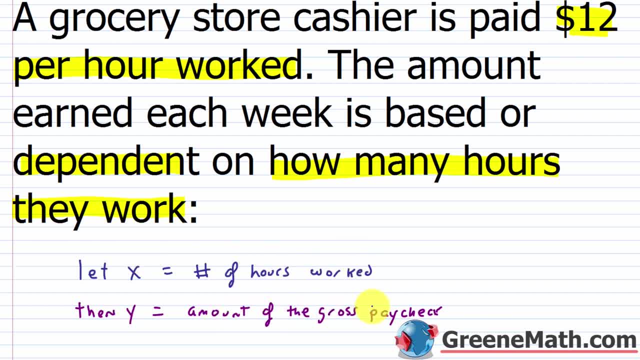 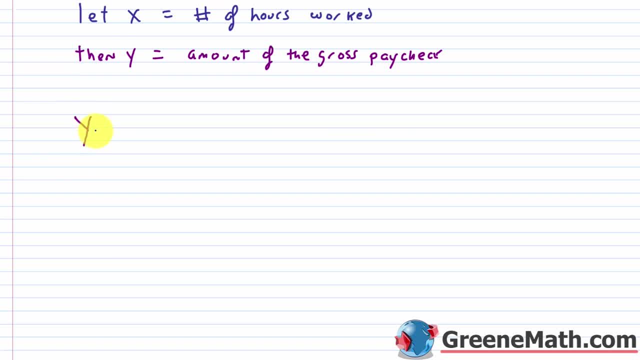 the number of hours worked, and I should get Y, which is the amount of the gross paycheck. So we have modeled this with an equation. So I'm going to say that Y is equal. Y is equal to 12X. Once again, this is the amount earned per hour. 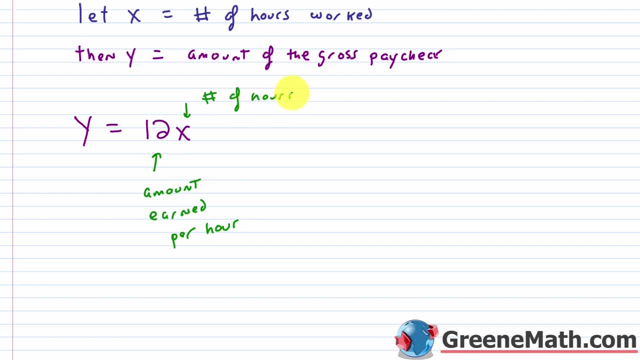 This is the number of hours worked. Again, you multiply those two together and you get the gross paycheck. Now, to make our example even simpler, Let's say that Let's say that the amount that she can work in a week could be zero or any integer value. 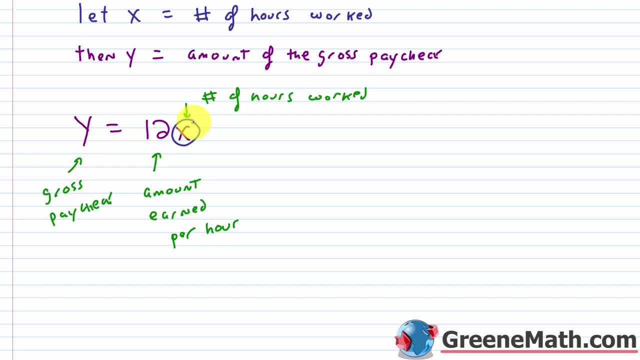 up to and including 40. So she could work zero hours a week. one hour a week, two, three, four, you know so on and so forth, up to the number 40. So for X it could be equal to: we'll represent this, starting with zero: one, two, three. 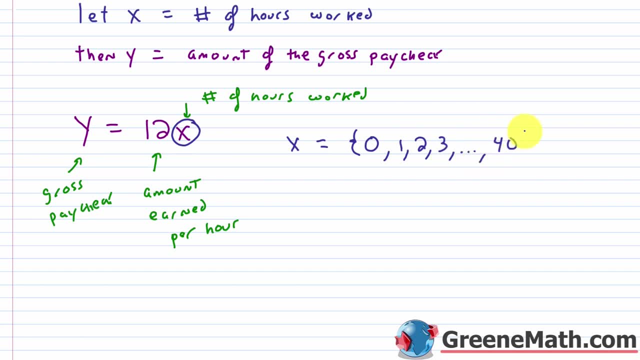 I'll put my three dots, And then I'm going to put my three dots And then I'll end this with 40. So any integer value including zero and including 40 and anything in between. So let's use this information to generate some ordered pairs. 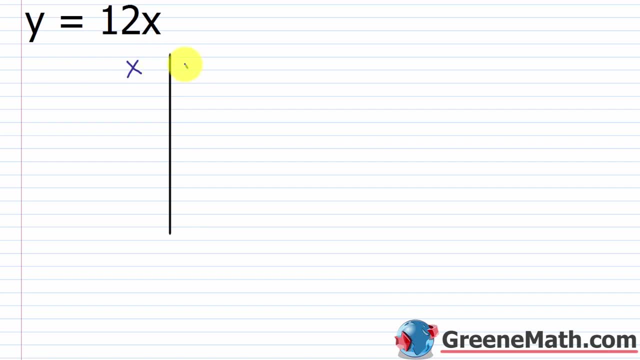 So I have here: Y equals 12X and I'm going to make a little table for ordered pairs. So again, X can be an integer beginning with zero and up to and including 40. So the first ordered pair, If I put a zero here. 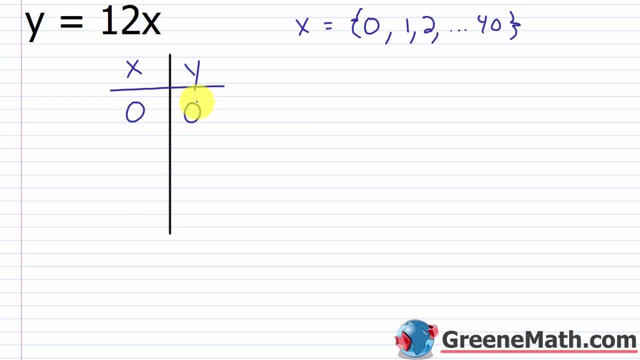 If I put a zero here for X, zero times 12 is zero And that makes sense. If I don't go to work at all or work zero hours, I would expect to make nothing. Now the next ordered pair: if I work one hour, I would get one times 12 or 12 for my paycheck. 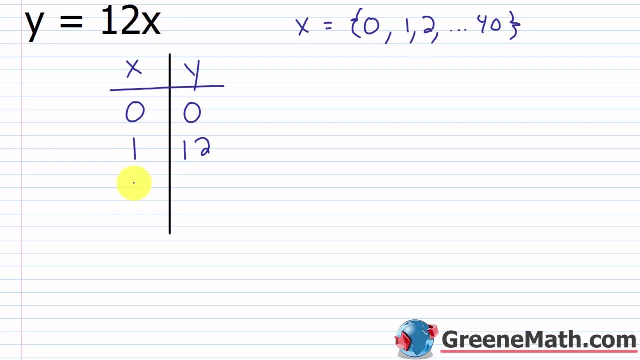 And we continue this. If I work two hours, two times 12 is 24.. And we would go all the way down. Eventually we get to 40 and that would give us what 40 times 12 is 480.. So 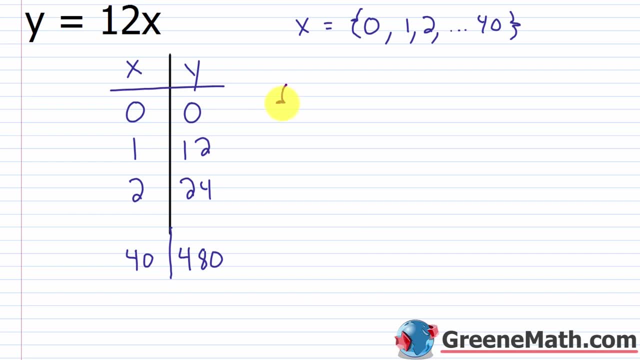 So this relation would look something like this. It's a set of ordered pairs, So we would have zero comma zero, We would have one comma 12.. We would have two comma 24.. Let's put our three dots and we'll put the final one, which is 40 comma 480.. 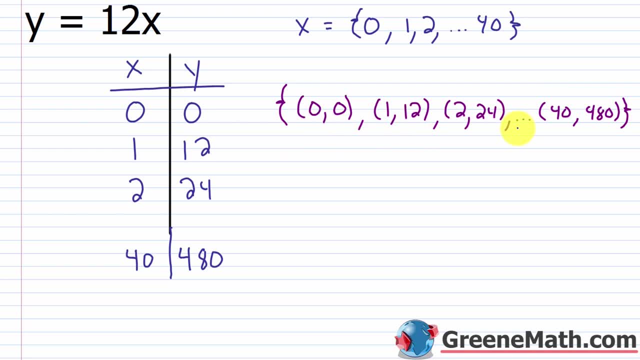 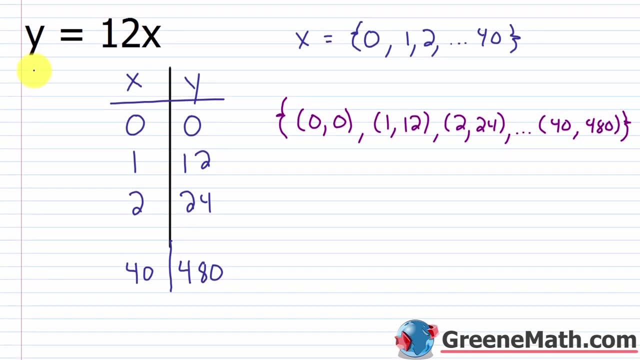 So this is a relation. Remember I told you, it's just a set of ordered pairs and these ordered pairs relate the number of hours worked to the gross paycheck in this scenario. So we can use this example to gain a few insights about relations in general. 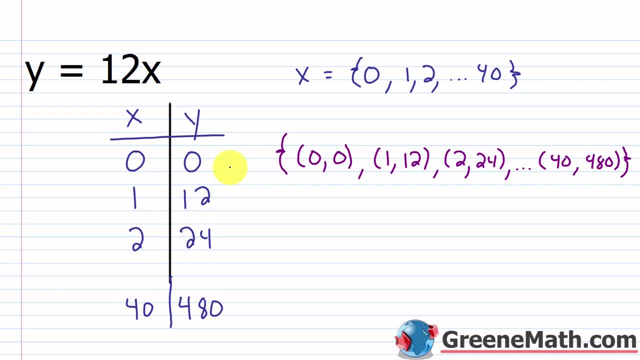 So there are two types of variables we're going to work with. The first type is called an independent variable or an input. for us, Generally, this is going to be X, So X, here is your input. The second type of variable is known as a dependent variable or output. 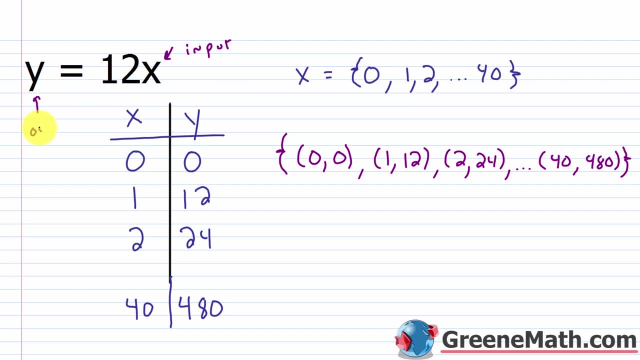 So Y is generally reserved. It's the output. So this is your dependent variable or your output. Now, why do we say independent variable or input? Why do we say dependent variable or output? Well, the independent variable is something you would choose. 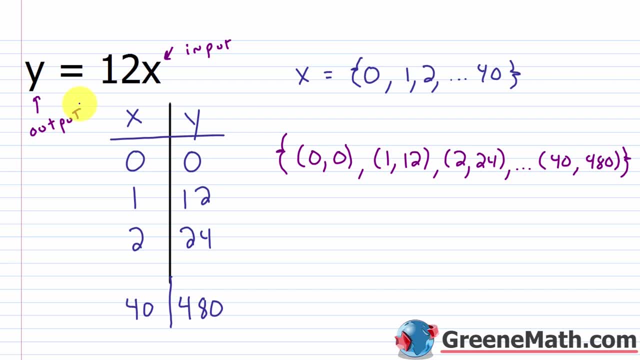 So let's say I'm a worker and this isn't- this isn't a hundred percent accurate, but typically I would choose how many hours I would work. right, I would say I make a choice of how many hours I would work and then I get a paycheck based. 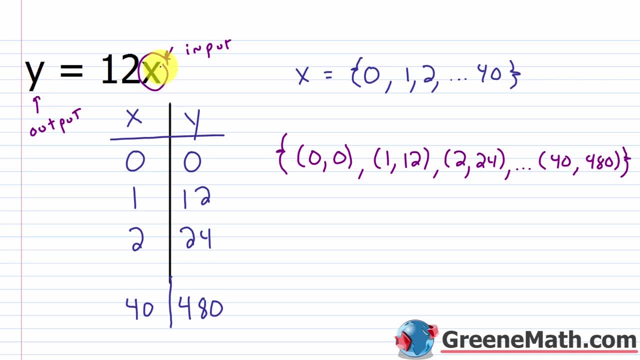 on that. So my independent variable is how many hours I work. My dependent variable is my paycheck. My paycheck depends on how many hours I chose to work And I know in the real world it's well, my employer made me work this or my employer. 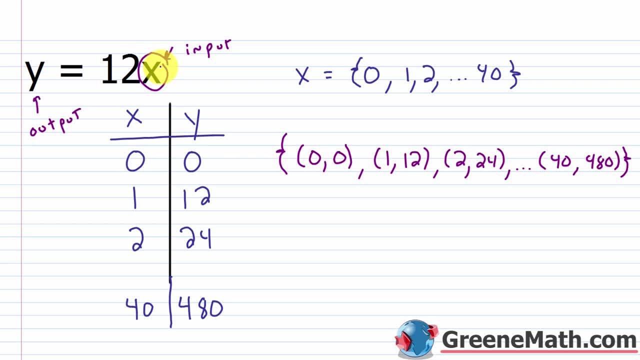 only let me work this. I get that, But let's just say there's a perfect scenario where you can choose any amount of hours you want to work. You can work between zero and up to 40 hours in one hour increments, All right. 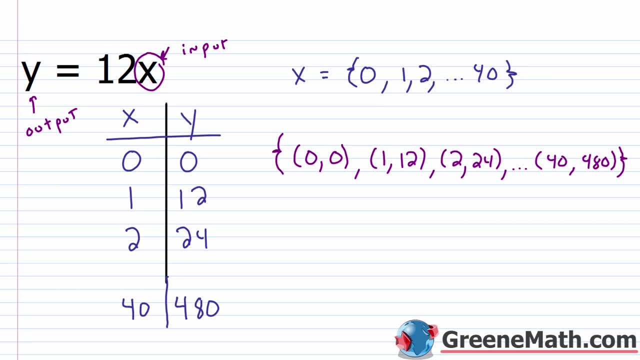 So there's two other things that we want to talk about. We want to talk about domain and we want to talk about range, And these are very important concepts for us and they're going to get super complicated as life goes on. in math, Right now, they're very, very easy to understand. 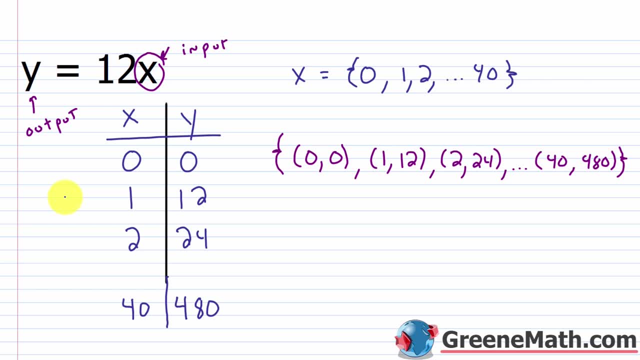 So a domain is just the set of allowable values for the independent variable or for X. So the domain in this case I told you was the set of integers starting at zero and going up to and including 40. So this would be your domain. 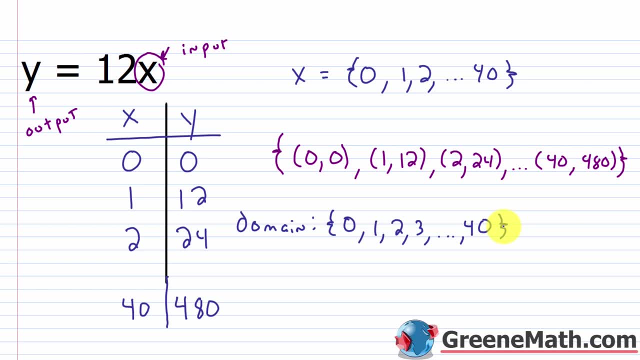 Then what would the range be? The range is a set of allowable values for your dependent variable, or Y. So the range in this case- and all we have to do is look at our equation- You think about what's plugged in for X. 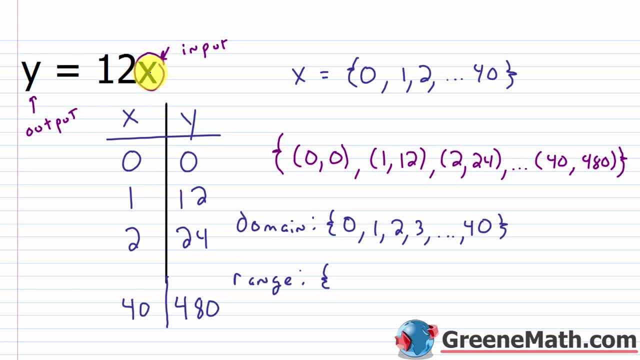 Well, I can plug in a zero, I can plug in a one, a two, a three, up to and including 40,, starting at zero, And then it's going to increment in multiples of 12.. So the next number would be 12,, then it would be 24,, then it would be 36,, right? 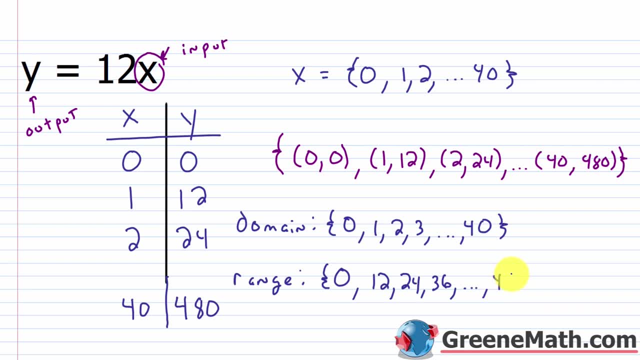 So on and so forth, up to and including the number 480.. You just have to list enough to where the pattern is clear. right, I'm increasing in increments of 12.. I know after 36 would come 48.. I know after 48 would come 60.. 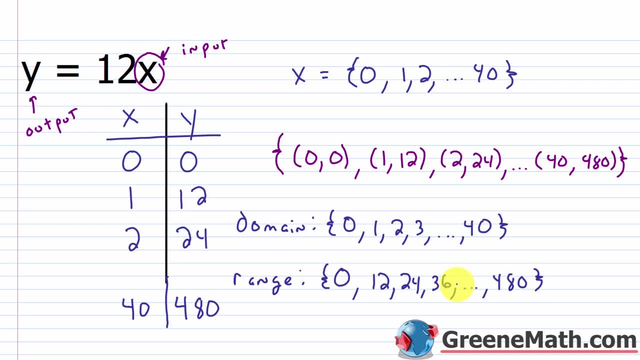 Then 72. Then 84, right, So on and so forth. So this is my domain and this is my range. So again, you got to remember for domain it's a set of allowable X values, or you might hear them say first components. okay, 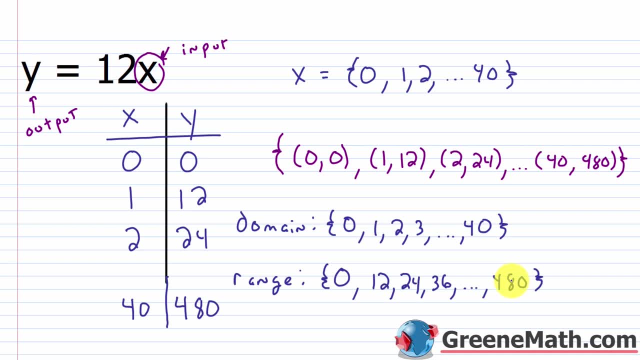 Because in an ordered pair, the first component is X, The range is a set of Y values, or second components, because in an ordered pair, the second component is the Y value. Let's talk about another real world relation that you'll come across. 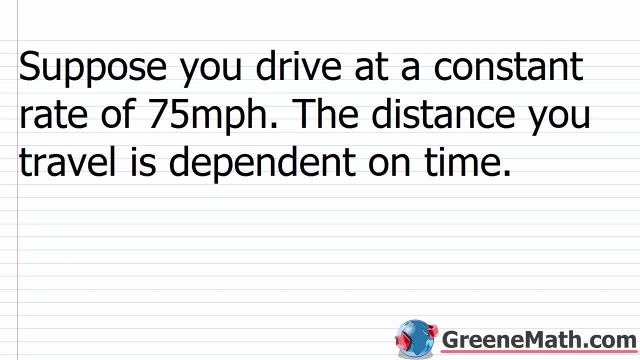 Suppose you drive at a constant rate of 75 miles per hour, The distance you travel is dependent on time. So we all know the distance formula right From working with motion work problems, we know that distance is equal to rate of speed multiplied by time traveled. 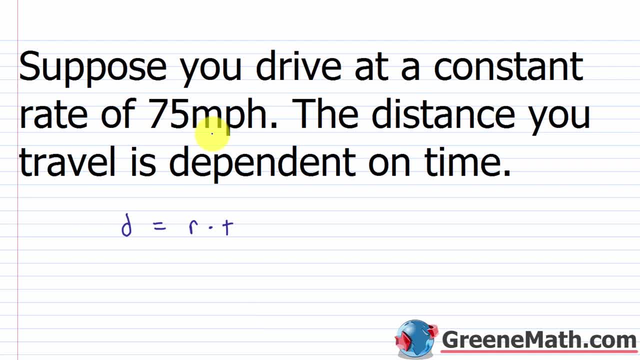 Well, in this case the rate of speed is given to us, It's 75 miles per hour. So distance is equal to 75 times time. Okay, And to use X and Y to make things clearer, we could say: let X be equal to the amount. 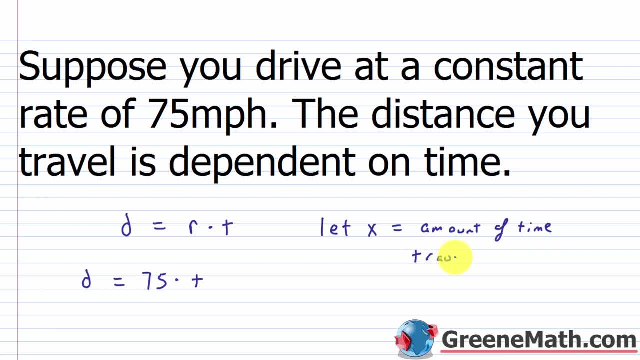 of time traveled in hours, And we could say: then Y would be equal to our distance, If we think about this. Okay, So T, here is the independent variable, which I'm replacing with X, just for simplicity. D- here is the dependent variable, which I'm replacing with Y, for, again, simplicity. 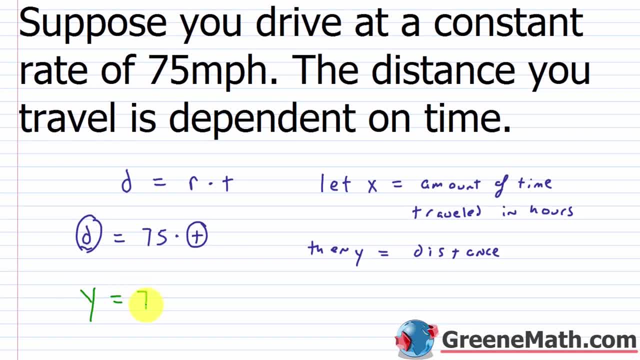 So I'm just going to write this equation: as Y equals 75X, So X is my input. I am choosing an amount of time that I'm going to travel for. Say, I'm on a road trip and I'm like: well, how long do I want to go today? 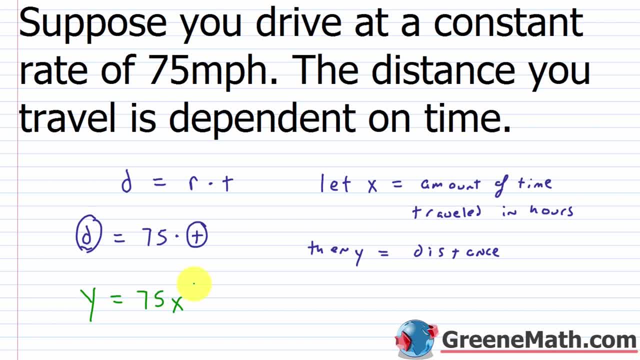 You know, I've got a certain number of miles, I've got a certain number of days to be there. So I'm going to go to a certain number of miles. I've got a certain number of days to be there. I've got a certain number of hours to make it over. 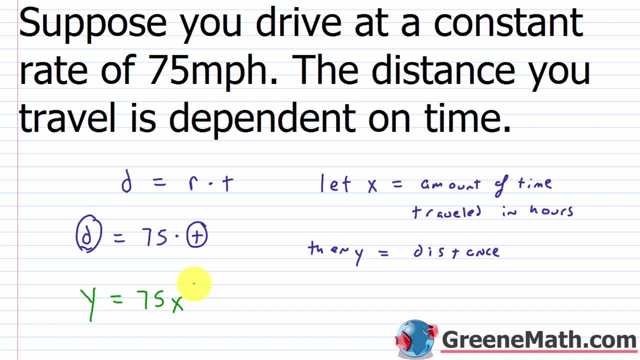 Do I want to drive for 10 hours, eight hours, six hours? How do I want to stretch out my trip? Well, I choose that value for X, I multiply it by 75 and I get a value for Y. So the distance that is traveled is dependent on the amount of time that I choose to drive. 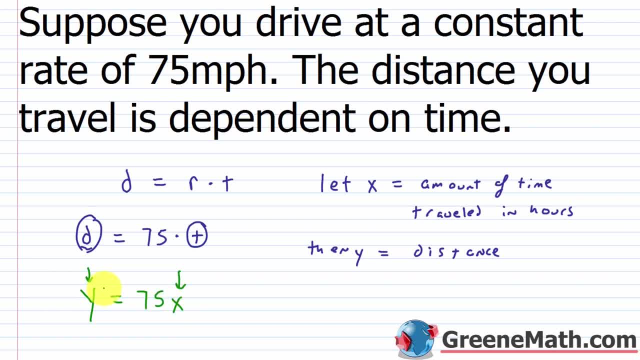 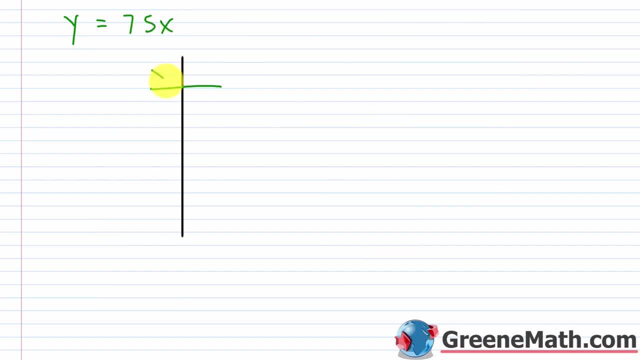 Okay. So again you've got your independent variable X, your dependent variable Y, So let's rewrite this: Y equals 75X And let's go ahead and make some ordered pairs for this as well. I'm going to say that X is going to take on a value that is an integer, starting with zero. 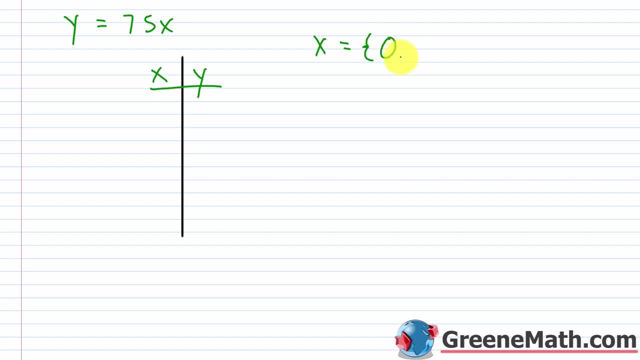 and going up to and including 10.. So we'll start with zero and go up to and include 10.. So that means X can take on these values. It could be zero, one, two, you know, so on and so forth till we get to 10.. 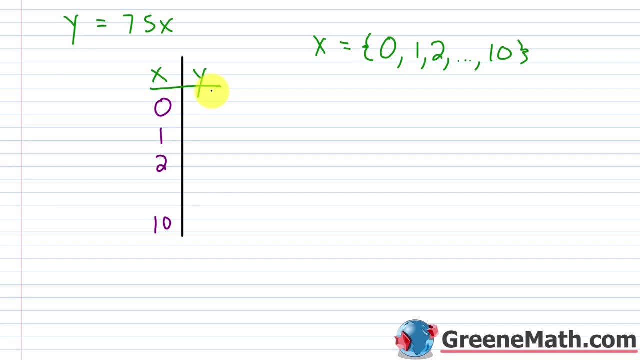 Y is obtained by taking X and multiplying it by 10. So that means X can take on these values. It could be zero, one, two, you know, so on and so forth till we get to 10.. Y is obtained by taking Y and multiplying it by 75.. 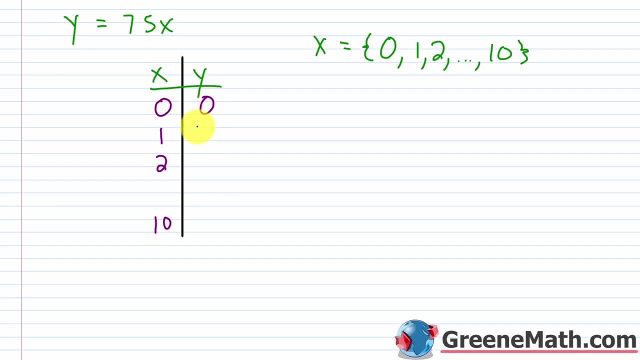 So here it's zero, and then we're going to increase by 75 each time. So this is 75, this is 150, you know so on and so forth, till we get to 10 times 75, which is 750.. 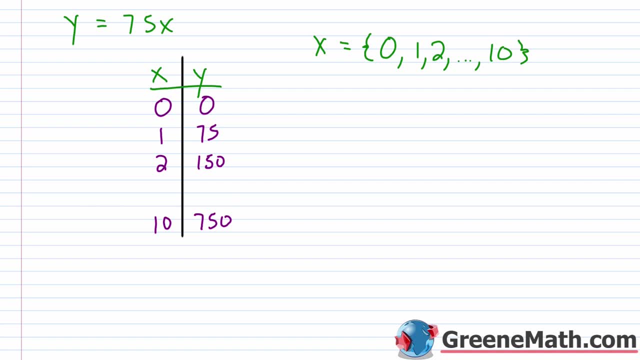 So if I think about my domain or my set of allowable X values, it's given to me right here. All right, I can choose to drive zero, I can choose to drive one, two, you know, so on and so forth. 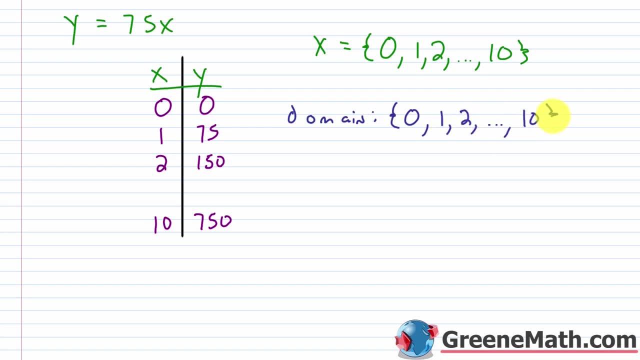 Up to and including 10 hours, So that's what I can choose as an input. I'm limited by my problem and what's told to me, and so I can't go over 10 hours. In the real world I can drive as much as I want. 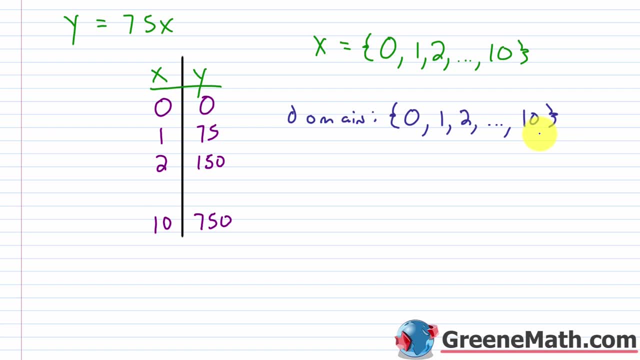 All right, I can drive till I fall asleep and crash into something. But for simplicity, I'm saying that you can choose not to drive at all, which would be zero, Or you can drive in increments of one hour up to and including 10.. 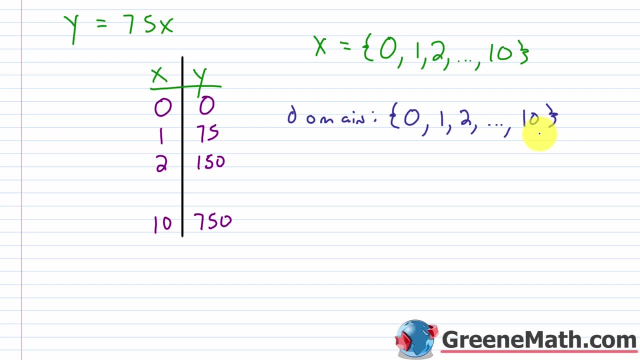 Right, So you can go up to and including 10 hours. So that's my domain. So what's the range? Well, the range is the set of allowable Y values. So think about plugging in each option for X. Well, I'd start with plugging in a zero If I drive for zero hours. 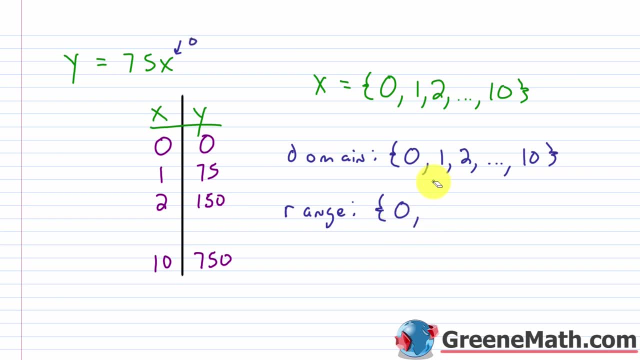 I go zero miles, not going anywhere, just sitting at the house. If I drive for one hour, I go 75 miles, And again I'm going to increase in increments of 75. So then I'm going to go to 150,. 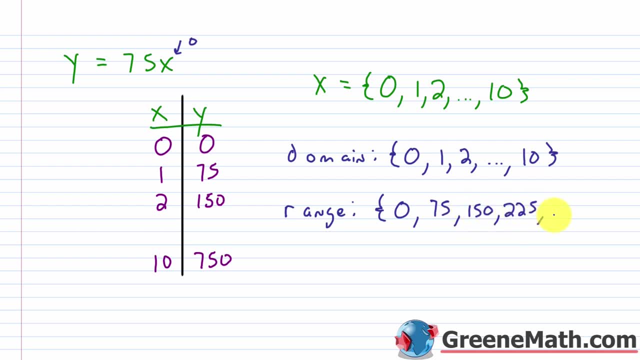 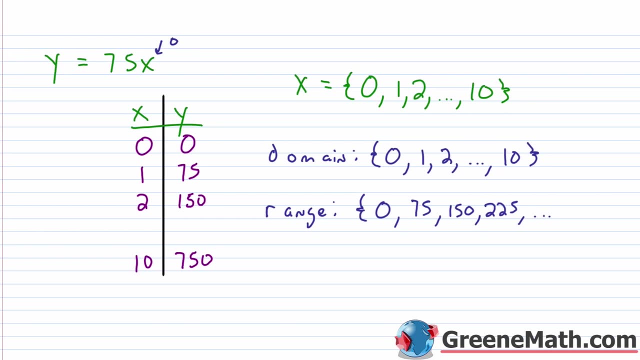 and then I would have 225, you know so on and so forth, till I get to the maximum amount I can drive, which is 10 hours, And in that particular case I'm going to go 750 miles, All right, 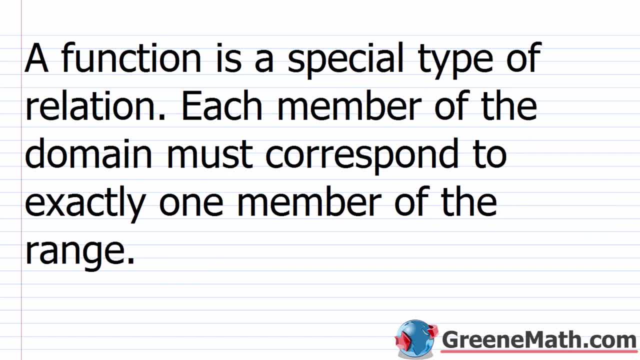 so, now that we've had two basic examples of a relation, again, this is how one quantity relates to another- Let's talk about functions, because that's really the purpose of this video. So a function is a special type of relation, All functions. 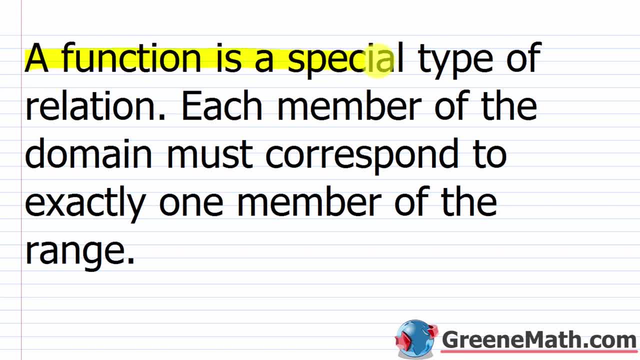 are relations. Let me highlight this. A function is a special type of relation. Each member of the domain must correspond to exactly one member of the range. So you might say: what in the world does that mean? That's super confusing. I want you to remember this. This is very easy. Each X value. 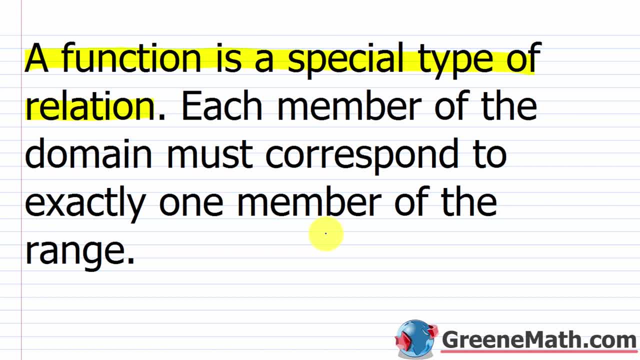 must correspond to or must be associated with or must link up to exactly one Y value. So if I give a function a function and I give it a function, and I give it a function and I give you something for X, it should be crystal clear what the output is for Y In this example. 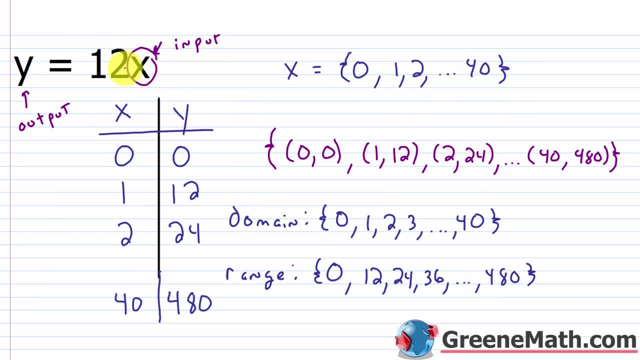 where we go back to the grocery store. cashier, if I choose something for X, I know what I'm getting for Y. If I choose, let's say, 40 for X, I know I'm getting 480 for Y. So there's a clear. 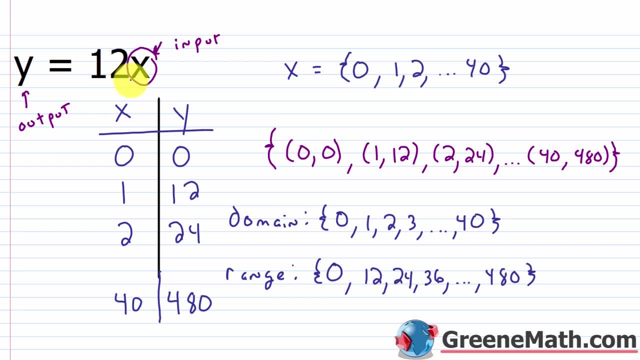 association. Every time I choose something for X, I know what the output's going to be. Now that sounds kind of silly, because we really haven't seen stuff yet where you choose something for X and you don't know what you're going to get for Y, But if you choose something for X, 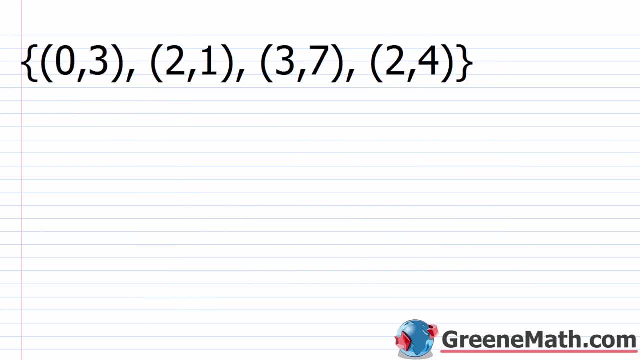 you're going to get something for Y, But I'm going to give you some examples here in a minute, So I want you to just to look at this set of ordered pairs here. When you first start looking at functions, these are the examples you get. They're super, super easy to deal with. All you're. 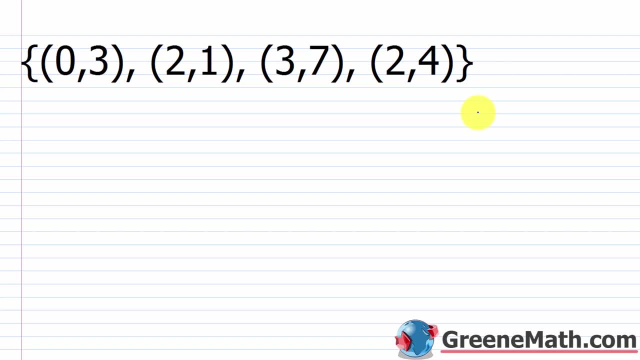 looking for here is duplicate X values. I'm just going to boil it down to that. If I look through my ordered pairs, I have 0,, 3,, 2,, 1,, 3,, 7, and 2, 4.. Do I have a duplicate X value? The answer to. 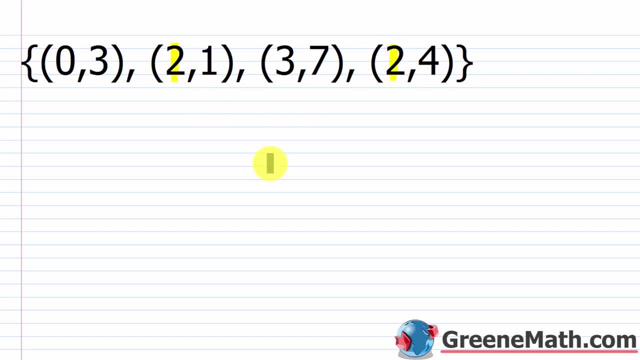 that is yes, I have a 2 here and a 2 here. This is not a function. Let me explain why, because some of you will probably be like: what do you mean If I think about X values here and I think about Y values? 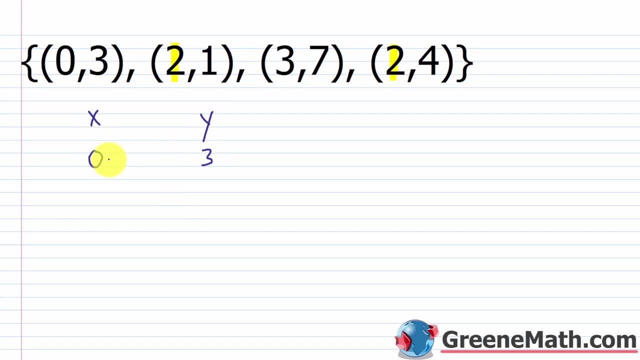 0 is my first X value. It is linked to or corresponds to 3.. So if I have an X value of 0, I know the Y value is 3.. There's a clear association. So that's fine, Let's skip over. 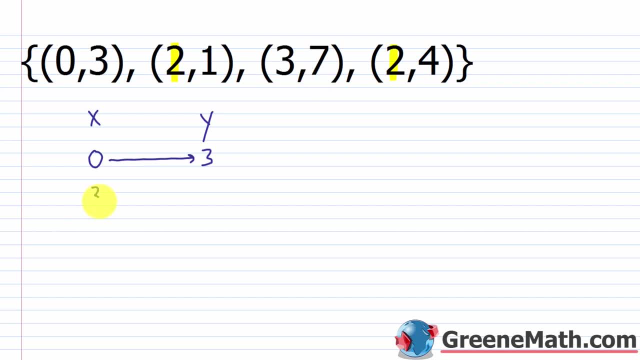 this for a second. Let's go to 3, 7.. Let's go to that ordered pair. So 3 is associated with or linked to, 7.. If I choose 3, 7, 7, or 3, 7,, I'm going to get 3, 7, 7, or 3, 7, 7, or 3, 7, 7, 7, 7,. 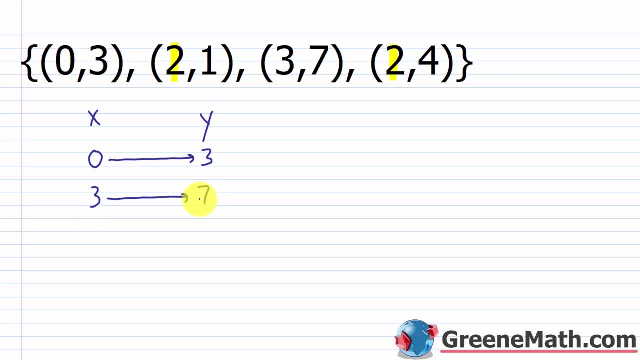 If I choose an X value of 3, I know I'm getting a Y value of 7.. Here's where there's a problem. I have this X value of 2.. I get a Y value of 1.. But I have an X value of 2 that also produces a. 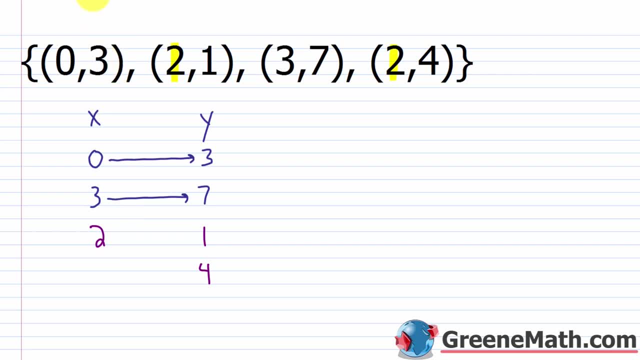 Y value of 4.. So it is unclear, if I have an X value of 2, whether my Y value is 1 or my Y value is 4.. There is no clear association there And as you get further in math, that's going to be a. 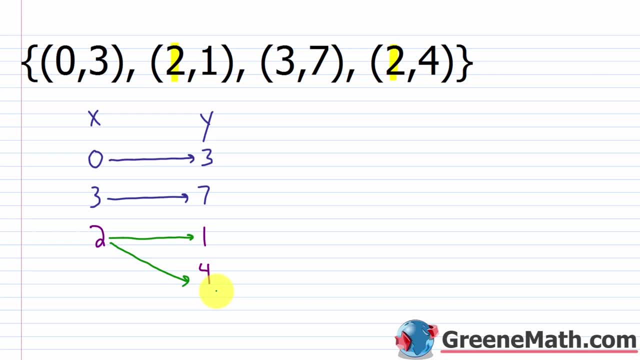 problem for you. If you have an X value of 2, you're going to get a Y value of 4.. So if I have an input, you expect one and only one output. If I choose an X, there should be exactly one Y. 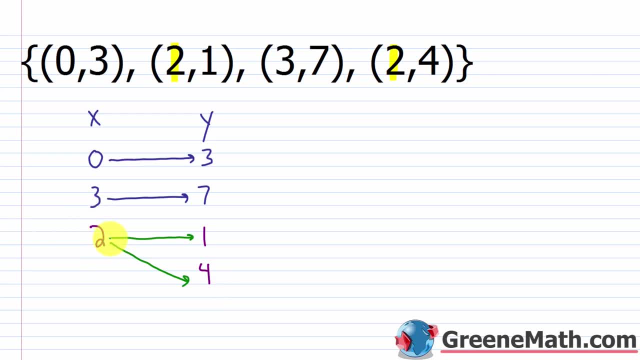 that is associated with it. Here I'm choosing an X value of 2, and there's two Ys associated with it, So this is not a function. Again, it's still a relation, but it's not a function- All functions. 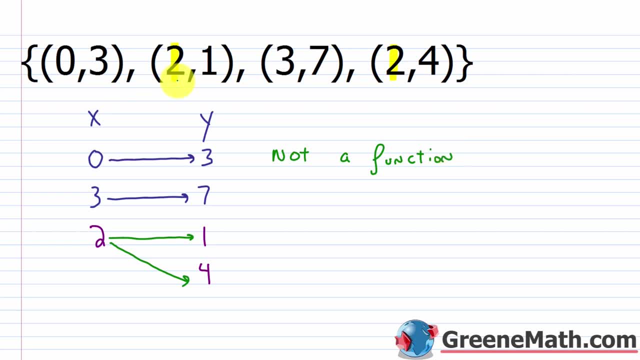 are relations, but not all relations are functions. Here you have a relation that is not a function. Let's look at another example. So we have these ordered pairs. here We have 3, 7, 2, negative, 6, negative, 5, 3, and 8, 4.. 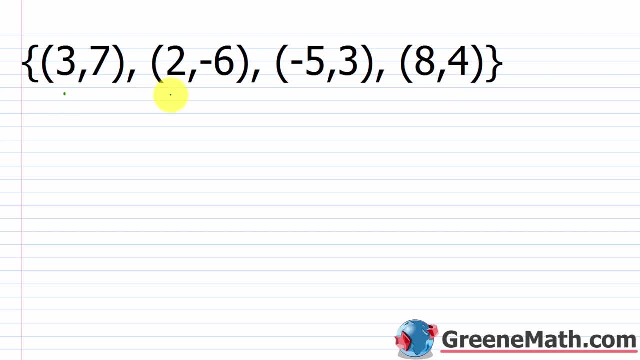 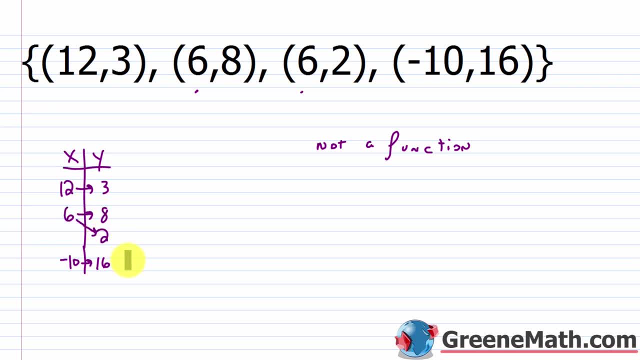 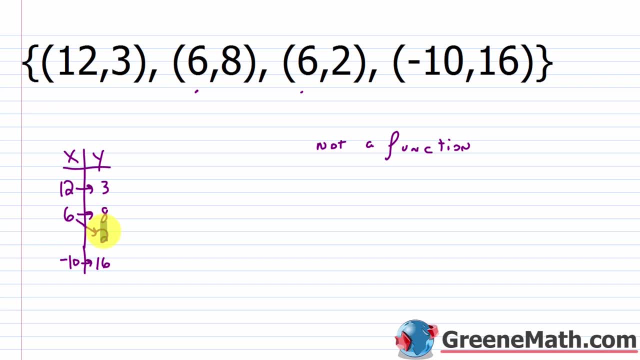 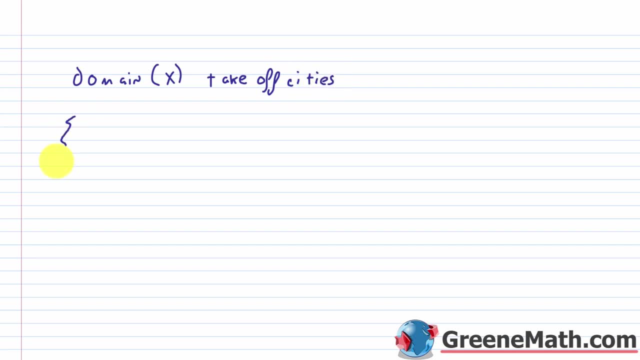 cities. So this is your domain And, to keep it simple, I'm just going to use three cities. Let's say there's New York, Let's say that there's Atlanta And let's say that there is New Orleans. Now, in my land of Y, that's my range. 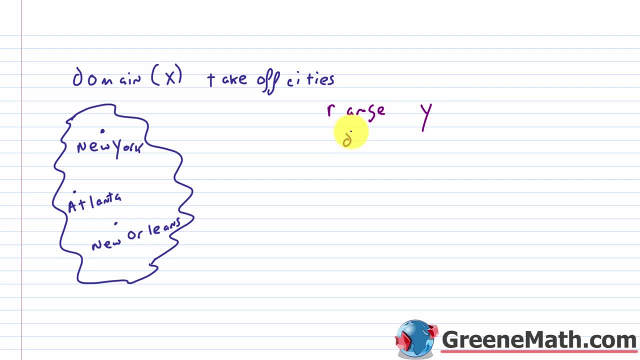 Okay, so my range is Y. This is the destination. Okay, so that's over here. This is my land of Y. So let's say that there's a destination of Los Angeles, Let's say there's Portland And let's say there's Tacoma. 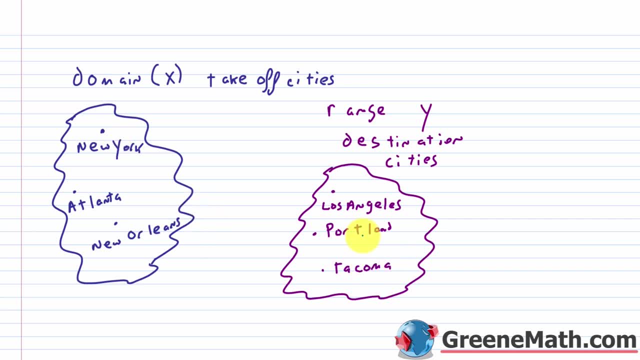 So think about X values as I'm taking off, Again Y values as destination cities or places that I will arrive. So for a function, there's a one-to-one correspondence. I leave from New York, I go to Los Angeles. I leave from Atlanta, I go to Portland. 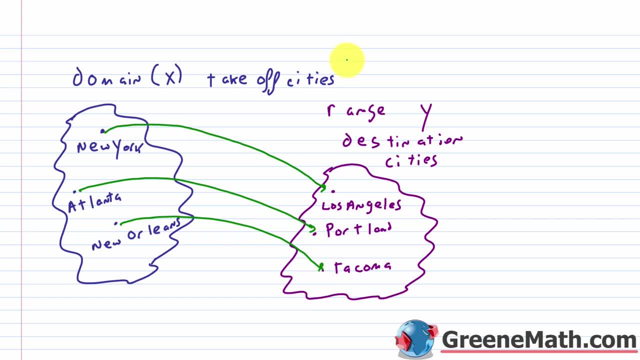 I leave from New Orleans, I go to Tacoma. So this is an example of a function. This is what we want, right? Because we say, hey, I'm leaving from New York, I need you to pick me up in Los Angeles. 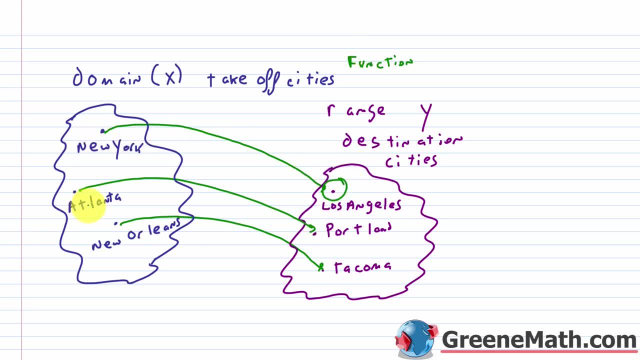 There's a clear association. I know where this flight's going to land. I'm leaving from Atlanta. I know I'm going to end up in Portland. I'm leaving from New Orleans. I know I'm going to end up in Tacoma. 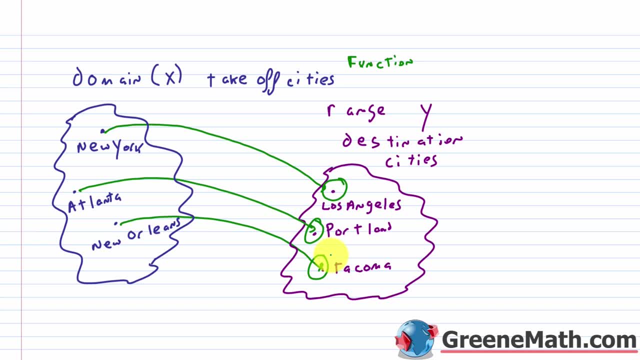 So this is a function. There's a clear association. What's an example where it's not a function? Well, let's say that the flight from New York is associated with Los Angeles and also Portland. Let's say the one from Atlanta is associated with Tacoma. 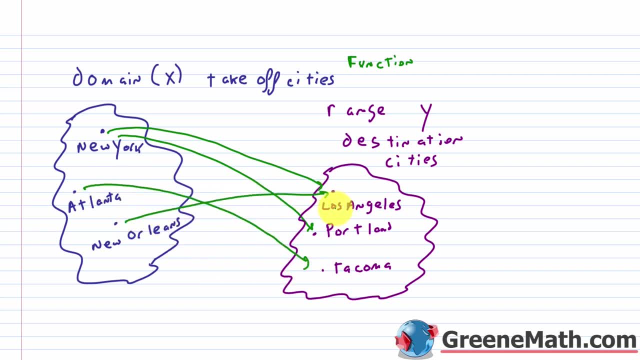 Let's say the one from New Orleans is associated with Los Angeles. Well, where there's a problem now is that this flight from New York is going to land in Los Angeles and it's also going to land in Portland. So imagine you get on this plane and you don't know where you're going to land. 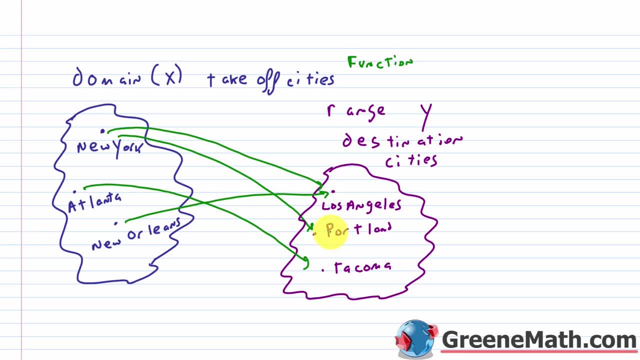 So you're calling people, You're like, hey, I might need you to pick me up in Los Angeles, but it also might be landing in Portland, So can you kind of call me right before I land? It's not a function, because 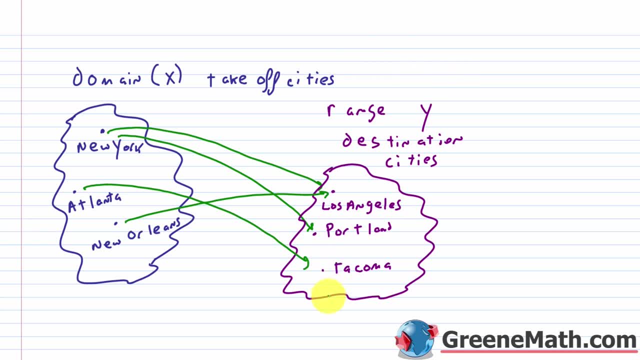 In this particular case, there's no a clear association. I have a value for x, which is New York, that is associated with two different values for y, Los Angeles and Portland. So it's not a function because there's no clear association. 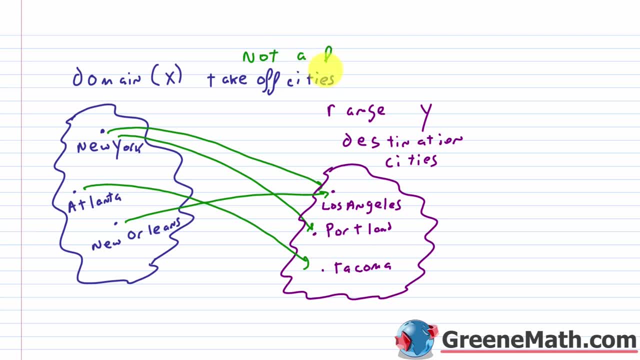 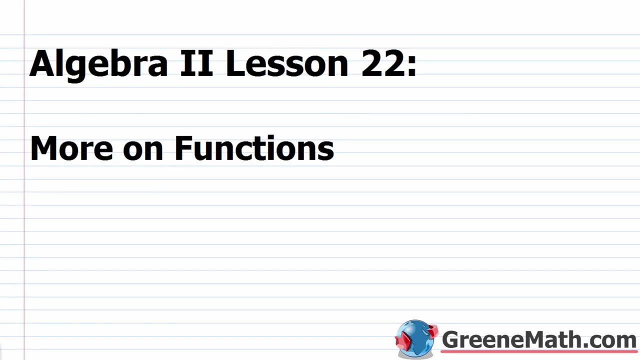 So this would not be a function. So not a function. Hello and welcome to Algebra 2, Lesson 22.. In this video we're going to continue talking about functions. So in our last lesson we talked about functions. In our last lesson we reviewed the basic definition of a function. 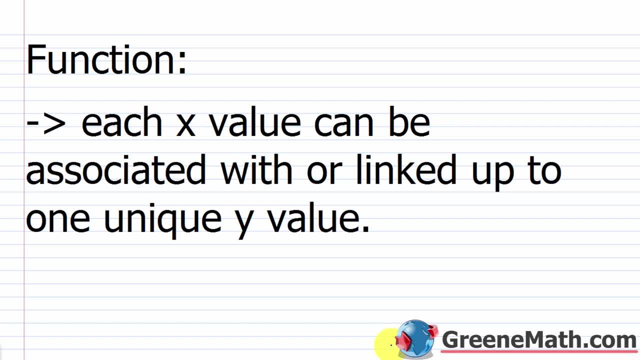 And when I say reviewed, if you took an Algebra 1 course, the last lesson that you went through here would be nothing new for you. We learned about relations in Algebra 1, and we also learned about functions. But just to give you a quick recap, a relation is nothing more than a set of ordered pairs. 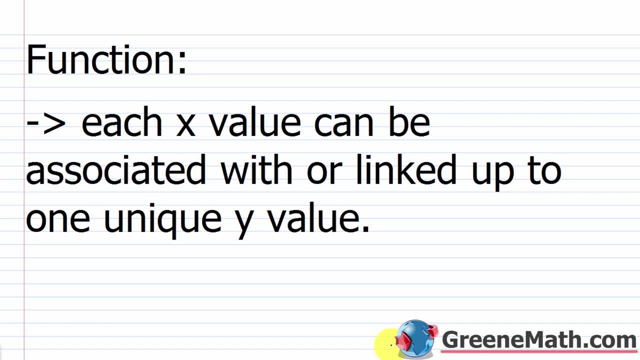 and a function is just a special type of relation, And I have here where each x value can be associated with or linked up to a function. So the common phrase you'll hear is: for each x there is one y. Now let's look at a quick example. 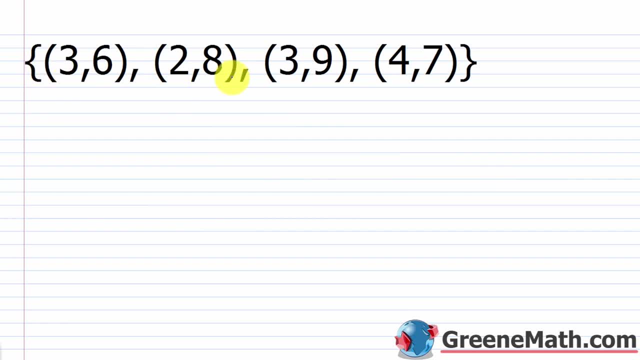 And this is something we saw in the last lesson, So I have a relation here, nothing more than just a set of ordered pairs. So we have 3,, 6,, 2,, 8,, 3,, 9, and 4, 7.. 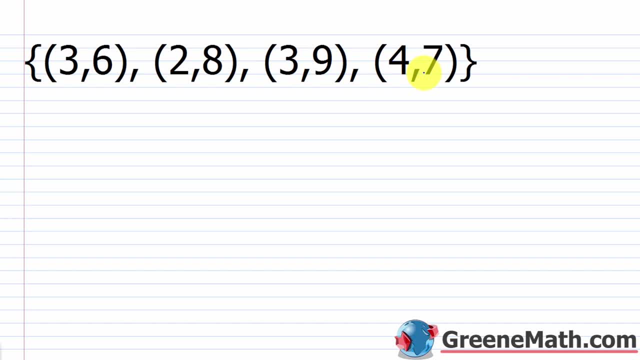 So the question I will put to you: is this a function or is this not a function? And it's really easy to see. So let's make a little table with x- y values. So if I have an x value of 3, I have a y value of 6.. 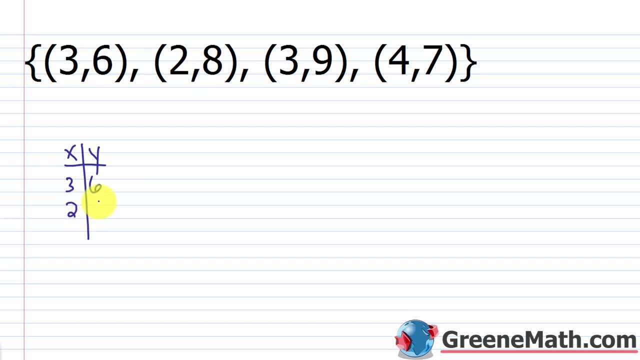 If I have an x value of 2,, I have a y value of 8.. If I have an x value of 3,, I have a y value of 9.. Well, I already had an x value of 3, and that was mapped to a y value of 6.. 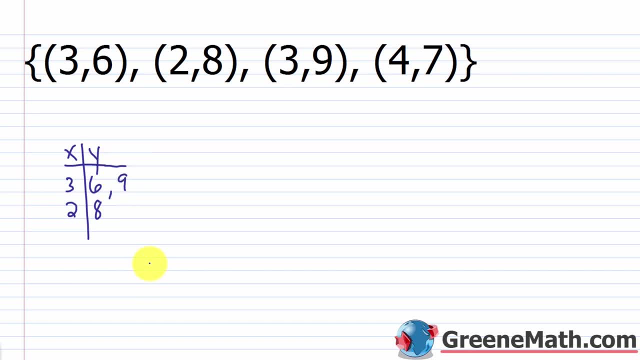 So let's just put 6, 9.. We'll talk about that in a second. And then, if I have an x value of 4,, I have a y value of 7.. I'll put the question to you again: Is this a function? 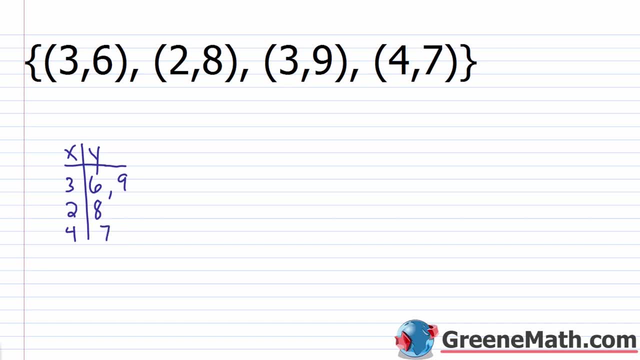 The answer is no, absolutely not. And why is that the case? Well, for each x, again, there can be one y, And you might pause for a minute and be like: what does he talk? what does that mean? Well, if I ask you, what is the value for y if x is 4 here? 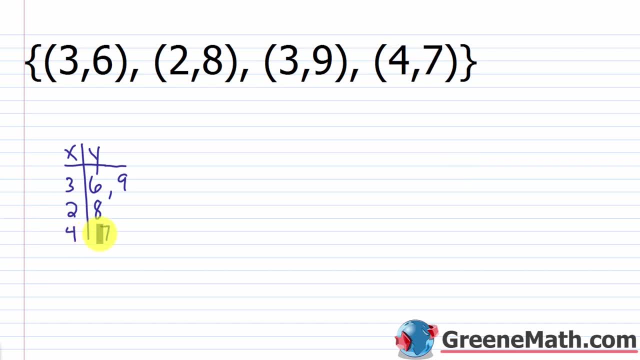 Well, if x is 4, y is 7.. Very clear. I can shout it out. If I say, hey, what's the value of y if x is 2?? Well, that's easy. y is 8.. 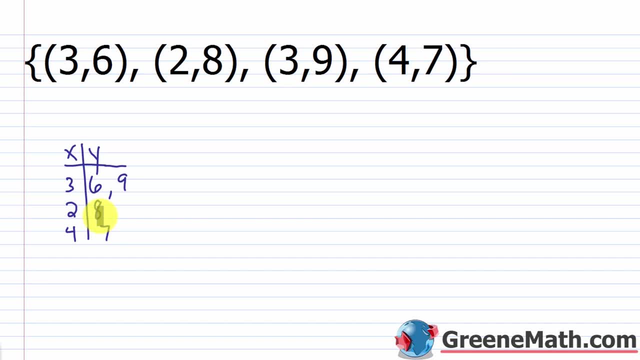 Now let me go to the one that's a problem. Let's say I say What is the value of y if x is 3?? Well, I don't know, It could be 6,, but it also could be 9.. 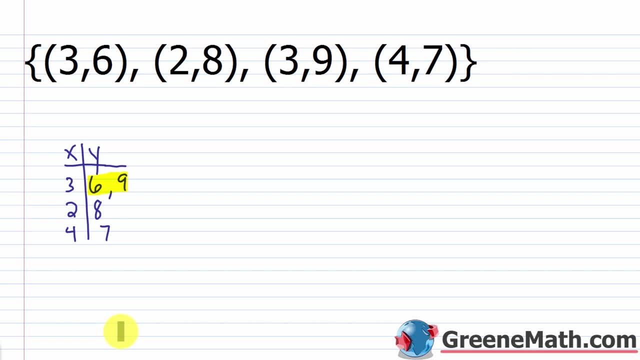 So there's no unique value for y, given the x of 3.. And that's the problem. That's why it's not a function: For each x value, you can have only one y value that corresponds to it. So for the x value of 3, I've got two y values that correspond to it. 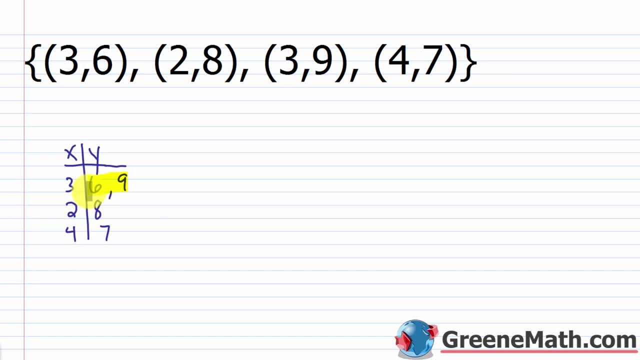 So that's why it's not a function. So that's what you need to be thinking about. If you get a simple example like this, it's really easy. I just go through and look for duplicate x values. I have an x value of 3 here and here. 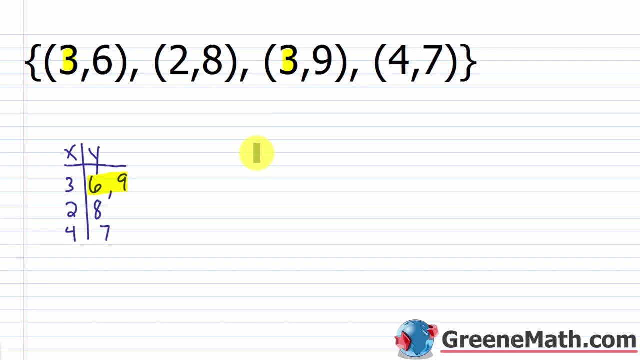 I already know it's not a function. That's really simple. The other thing: that kind of trips students up. Let's say you had another set of ordered pairs. Let's just erase this real quick. Let's just say I was looking at this set right here and it was 6, 2.. 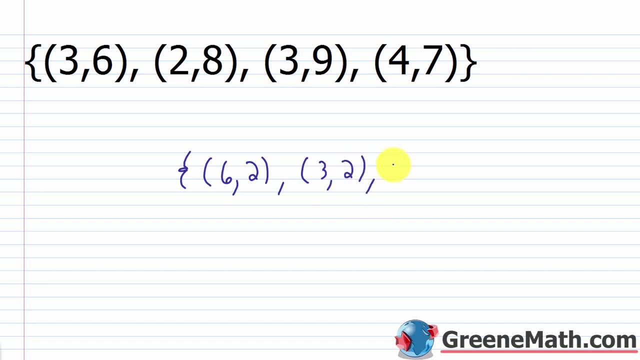 And let's say we had 3,, 2.. And let's say we had 4, 7.. Something like that. Is this a function? Yes, it is. And you might say well, no, no, no, no, no. 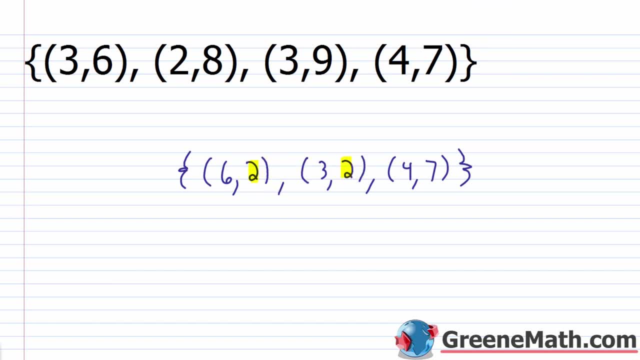 There's a 2 here and a 2 here. Well, let's look at it. Let's go through the same reasoning. Here's the x, Here's the y. So an x value of 6 is corresponding to a y value of 2.. 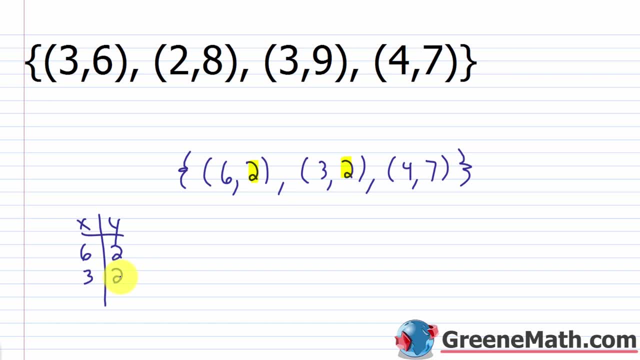 An x value of 3 is corresponding to a y value of 2.. An x value of 4 is corresponding to a y value of 7.. So for every x I have, I have exactly one y. It doesn't matter that different x's correspond to the same y. 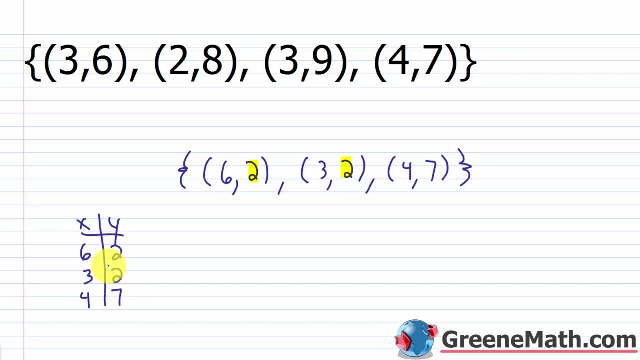 That's okay. It's just a matter of if I say, hey, what is y when x equals 6?? There's a clear answer: It's 2.. What is y when x equals 3?? There's a clear answer. 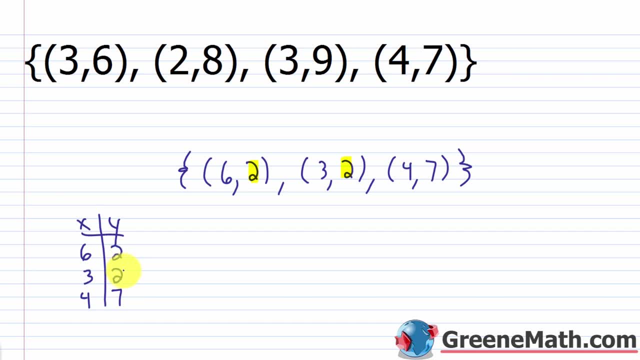 It's 2.. What is y when x equals 4?? There's a clear answer: It's 7.. So that is the difference at the most basic level of what a function is and what a function is not. Now let's turn up the heat a little bit. 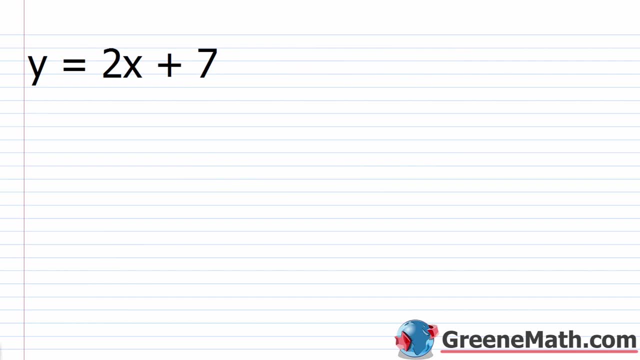 So we're done with the algebra 1.. Kind of easy stuff. Let's move on into the algebra 2 stuff. So you're not going to get a set of ordered pairs kind of driven to you, You're not going to get spoon-fed this stuff anymore. 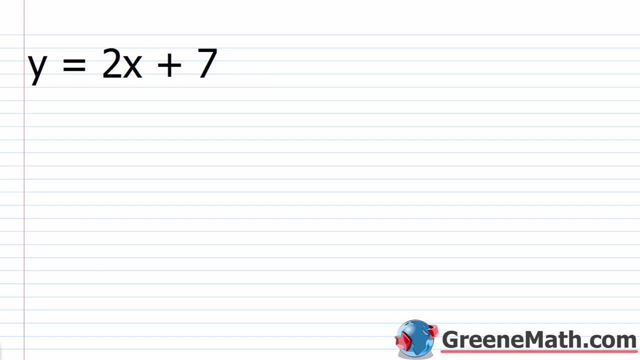 Now you're going to have to look at equations and say: this is a function, This is not a function, So it gets a little harder. So what are the tools that we can use for this? Well, one tool I'm going to give you is to graph. whatever you're looking at. 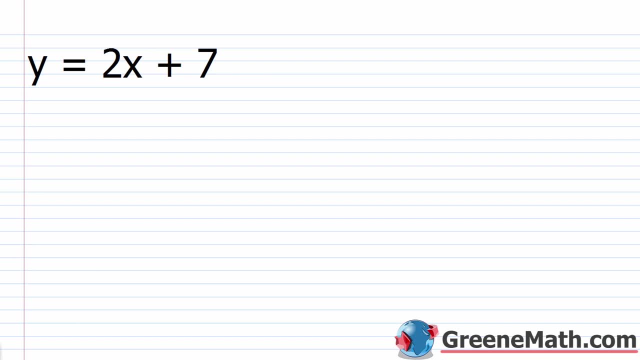 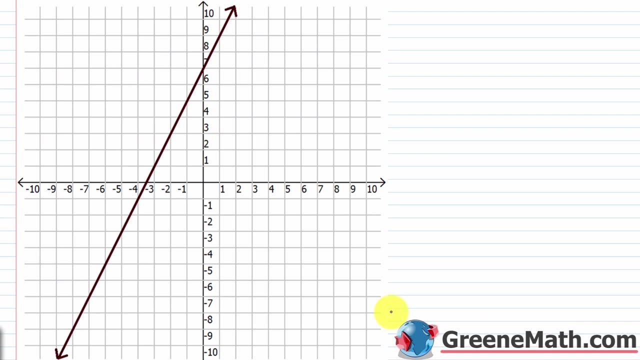 And you're going to use something known as the vertical line test. So I'm going to start out with y equals 2x plus 7.. And I want to look at this on a coordinate plane. All right, So let's take a look at the graph of y equals. y equals 2x plus 7.. 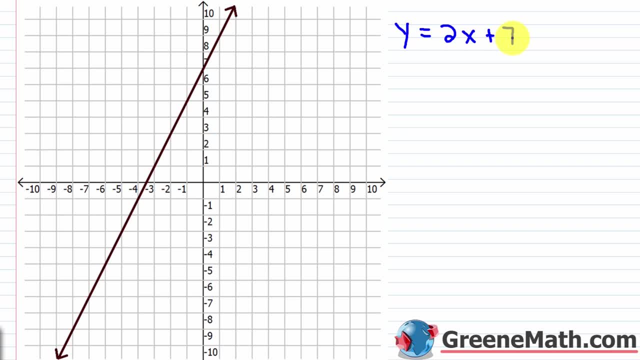 And we're going to determine if this is a function or not by doing something known as the vertical line test. So what is the vertical line test? Well, the vertical line test tells you if you have a function or not, based on if any vertical line will impact the graph in more than one location. 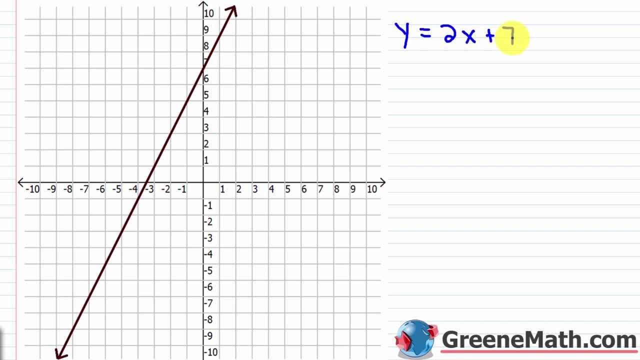 You might say: well, why would that work? Well, think about vertical lines for a second. by their nature, If I give you a vertical line and let's just say I wanted to graph, x equals 8, just as an example. 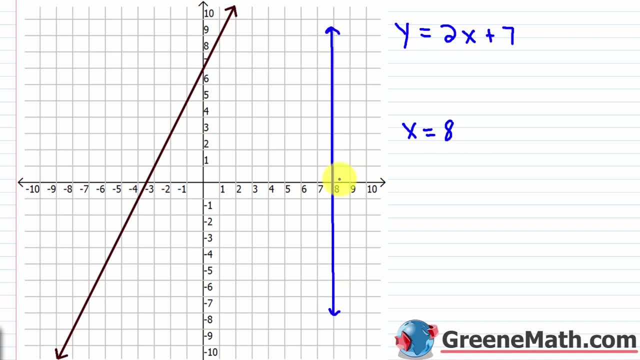 So for x equals 8,. I know that x always is 8.. The y values will change, but x always equals 8.. So for a given x value, I have many, many, many y values, an infinite number of them. 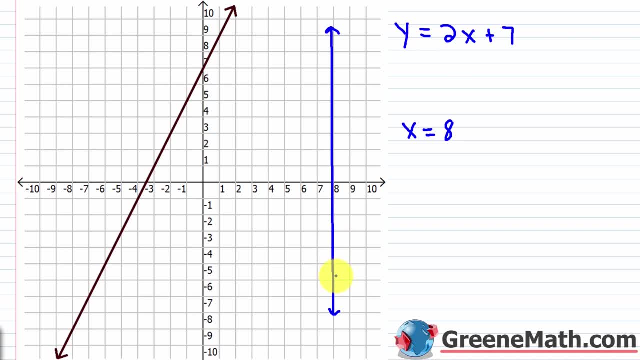 So if a vertical line, If a vertical line touches this one, were to touch a graph in more than one location, let's just say, for example, I had something that looked like this: Well, if it impacts it here and here, well, that means I have two different y values for that given x value. 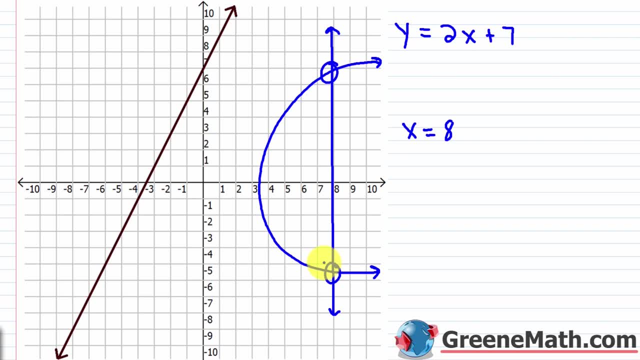 So that is not a function. That's where this vertical line test is going to come into play. Now let's erase this for a second And let's just think about what we have here. We have y equals 2x plus 7.. 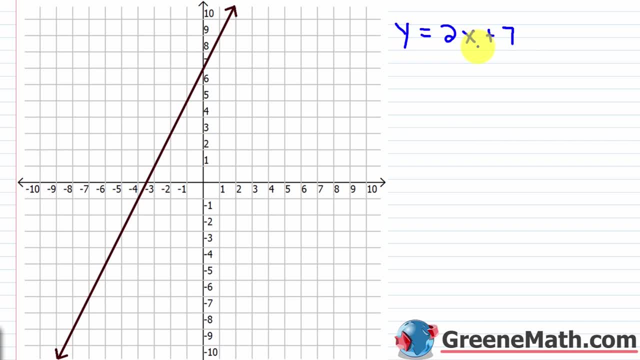 If I drew a bunch of vertical lines- and I wanted to- would I ever hit the graph more than once? Let's just draw three of them just for fun, So you can look at the lines I drew and in each case they only impact the graph once. 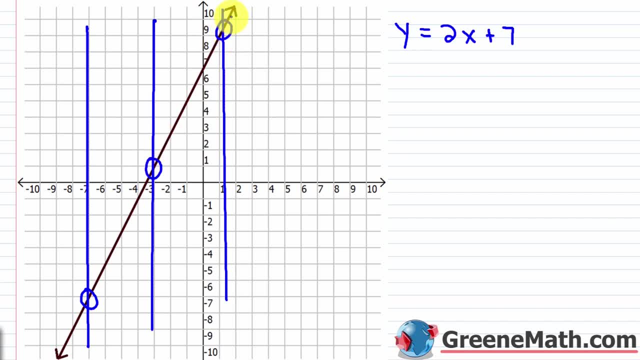 This one impacts it here, this one here, and this one here, And I could draw as many vertical lines as I want. in this case, This is the graph of a function. So y equals 2x plus 7 is a function. 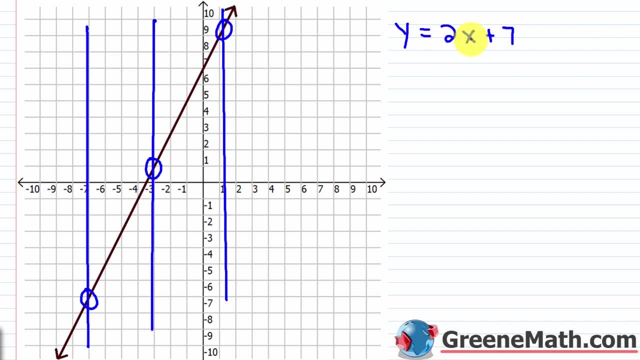 In fact, any time you get a linear equation in two variables, unless you have a vertical line, something like x equals some value, it's always going to be a function, right. And why is x equals some value not a function? Well, as I just showed you, 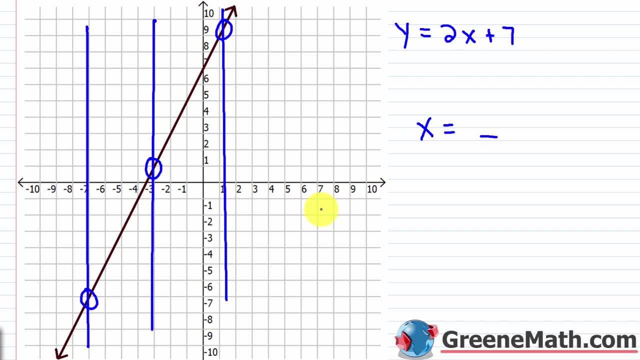 when I graphed, x equals 8, for that one x value, you have an infinite number of y values. so that is definitely not going to be a function. okay, But anything else that you come across, even if it's a horizontal line. 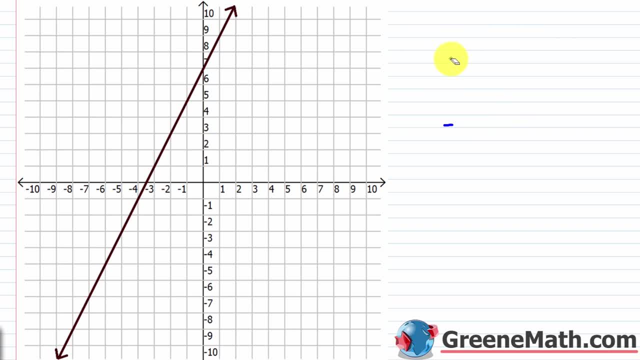 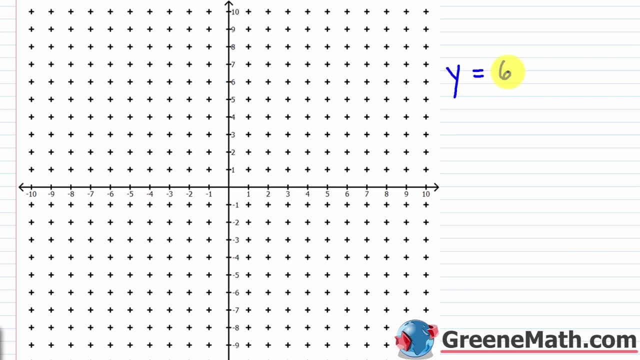 you know, if I erase this and I got out, let's say, a blank sheet and let's say I graphed: y equals 6, as an example, Well, I would go to the y axis and I draw a horizontal line through 6.. 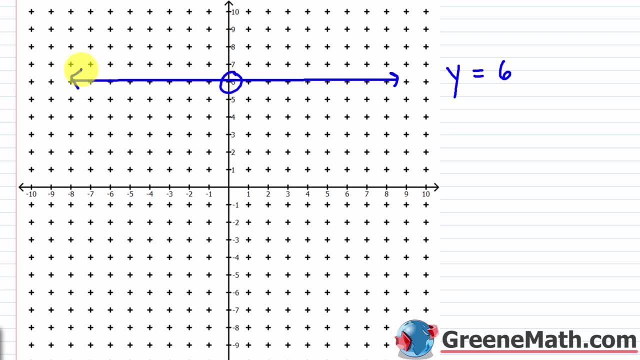 So I'll put the question to you: Is this a function? The answer is yes, Because for every x value- say for an x value of negative 2, I get a y value. It doesn't matter that it's the same y value. 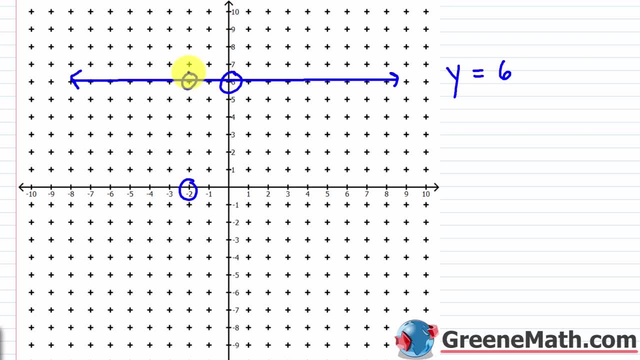 It doesn't matter, matter what x value I choose, I always get y equals 6.. But for each x I just get one answer. I don't say: well, x is negative, 2, y is 6, and then something else, It's only 6.. So for every x value there is, 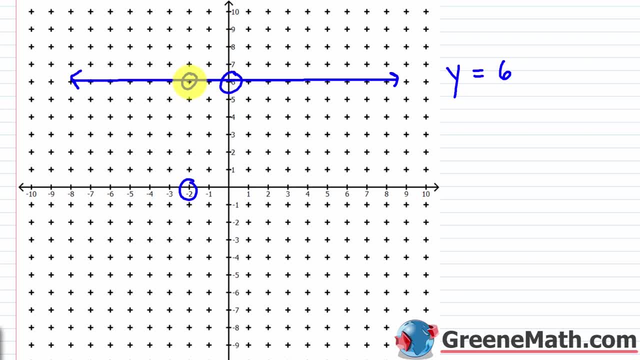 one y value. So this meets the definition of a function. So every linear equation in two variables that you come across is going to be a function, with the exception of when you get x equals some value. That is not a function. So only a vertical line is going to fail, All right. so I want to talk. 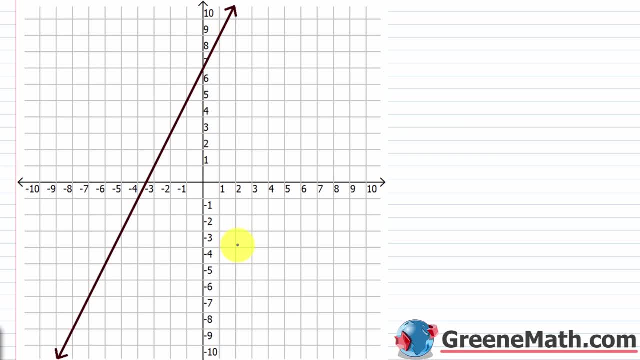 a little bit more about domain and range while we're looking at this picture. So what is the domain here? The domain is the set of allowable x values. So we can get that from the graph or we can kind of look at the equation and figure out. If I look at the graph I see that. 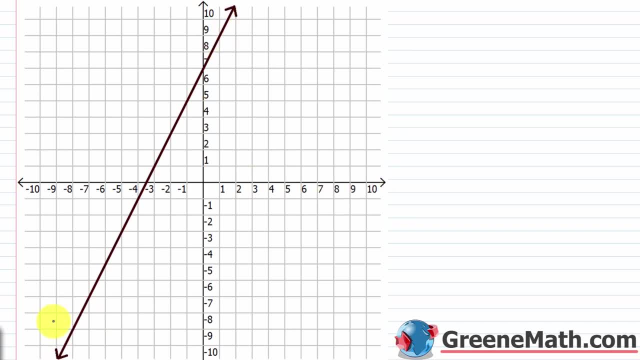 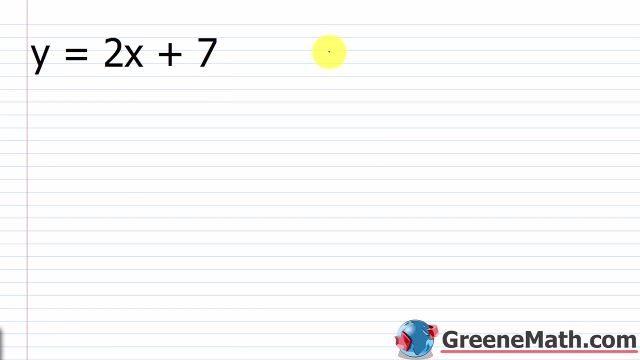 the x values here. well, because of the arrows there, that tells me this continues indefinitely in each direction. So for the x values, for the y values, I know that they're infinite in each case, Right, basically, from negative infinity to positive infinity. And if I go back and I look at my equation here, I could figure that out. And how would I go about? 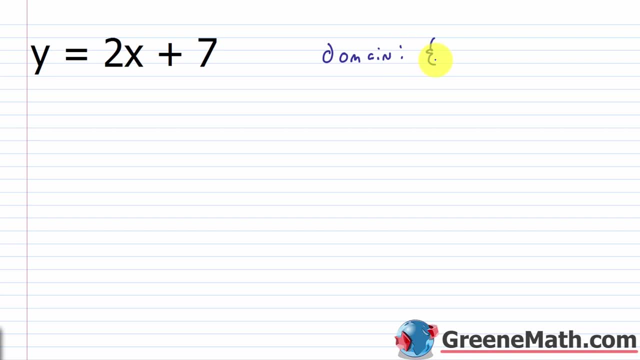 doing that. Well, what I would say is that: what can I plug in for x? What would be a possible restriction? Can I plug in a negative? We'll try it. If I plugged in a negative 2 there 2 times negative, 2 is negative 4.. Negative 4 plus 7 is going to be 3.. I could plug in as small of a. 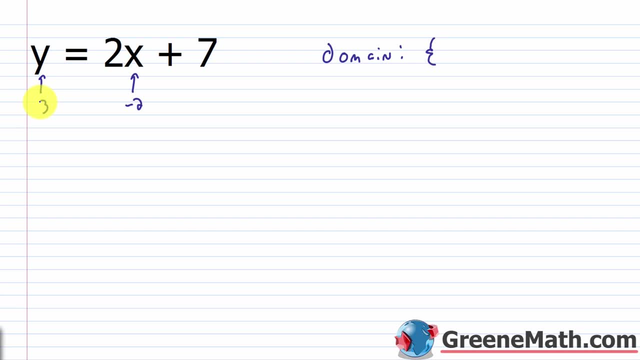 number as I want, Meaning a really, really, really big negative number, like negative 1 billion. I could go as large of a negative as I want, which means a really, really, really, really, really small number. So that is okay. I could go down to negative infinity. What about 0?? Could x be 0?? 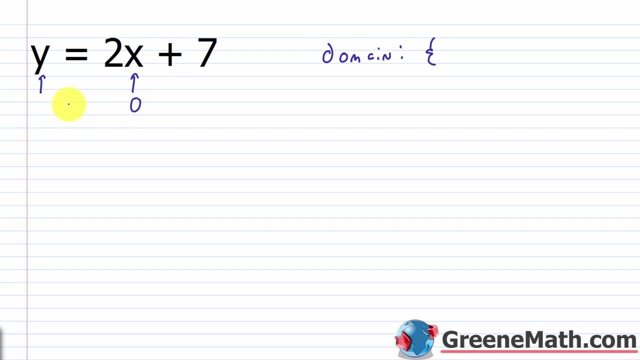 Yeah, x could be 0.. 2 times 0 is 0.. 0 plus 7 is 7.. That's okay, The world hasn't blown up. Everything's fine. What about a positive value? Yeah, I could. I could make x positive 2.. I could have x of 3.. 2 times 3. 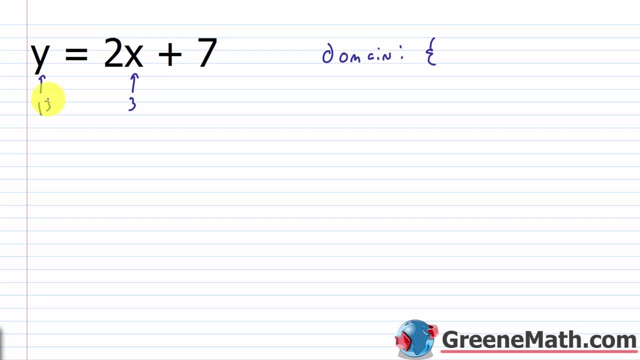 plus 7 is 13.. So that's okay as well, And I could go out to positive infinity. So x can basically be any real number, right? So I could write the domain as all real numbers, like this. I could also write this: an interval notation from negative infinity to positive infinity, like that. What about the? 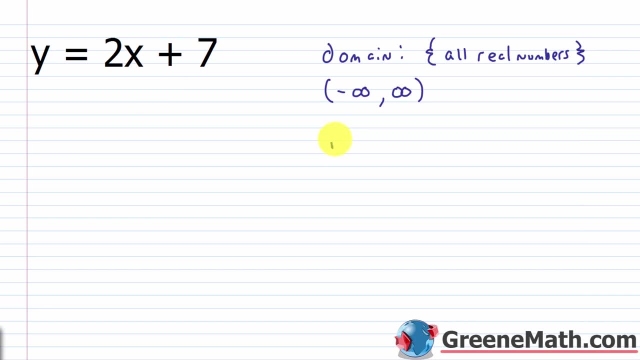 range. What is y allowed to be? Remember: we think about this in terms of input output. X is your input, Y is the output. So I plug something in for x, I get something for y. That's how we have to think. 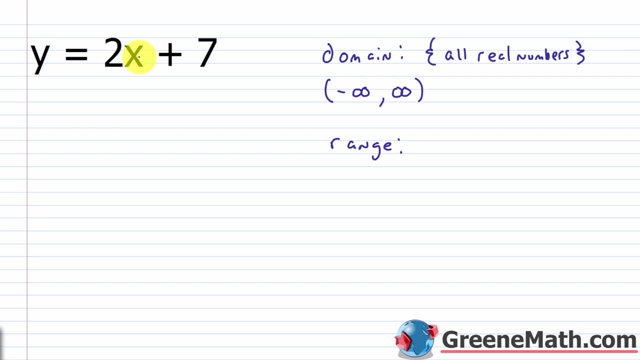 about these things? Well, can y be whatever I want it to be? The answer to that is yes, I can make it as small as I want. I can make it 0.. And I can make it as large as I want just by varying x. So the 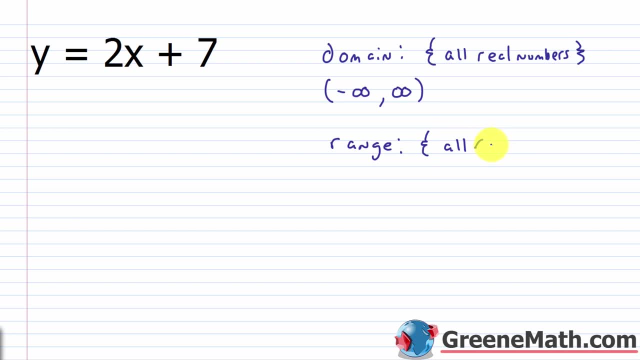 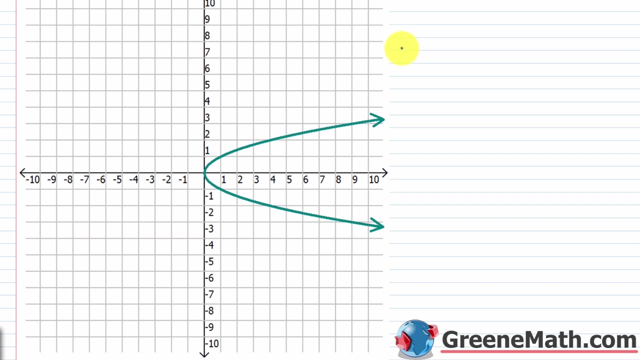 range is going to be all real numbers as well. So an interval notation again, from negative infinity to positive infinity. Alright, let's look at one that's a little bit more challenging. So we have: y squared equals x. So I'll put the question to you before we look at the graph: Is this a function? So, again, this is y squared. 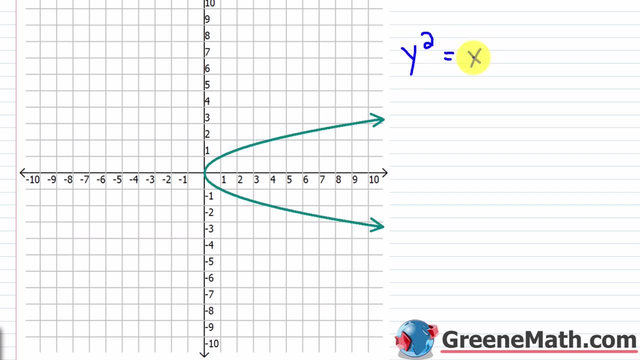 is equal to x. Does this look like the graph of a function? No, it does not Why? Because if I use my vertical line test, I'm going to find that a vertical line will impact the graph in more than one location. Let's just take 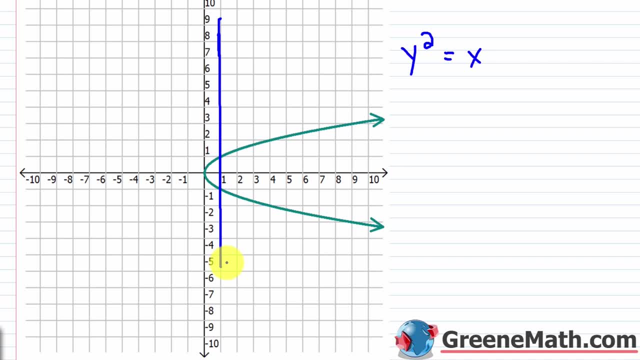 this one. So I draw a line where x is equal to one. So if x is one, what could y be? Well, it shows us here that y could be one and here that y could also be negative one. Does that make mathematical sense? 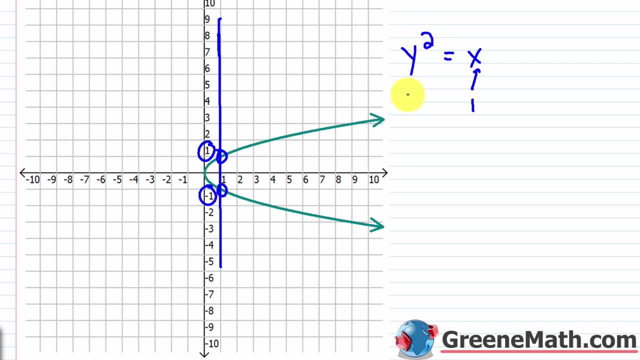 Well, yeah, I've got this squaring operation going on. So that means if I take one, one squared would give me one That works. If I take negative one and I square, that Negative 1 squared will also give me 1.. 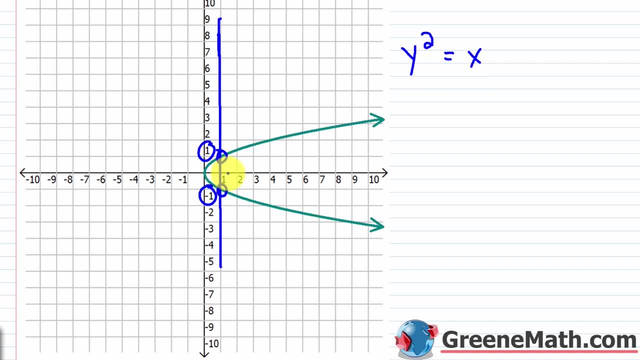 So that's why this is not a function For each x. there's not just one y For an x value of 1, I've got two y values that are associated: 1 and negative 1.. I take another example of 4.. 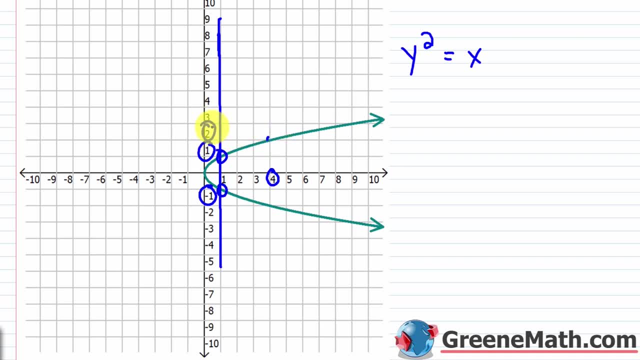 I've got two y values associated. You've got 2 and negative 2.. I take an x value of 9 as another example. I've got 3 and negative 3.. Again, it's because of that squaring operation. 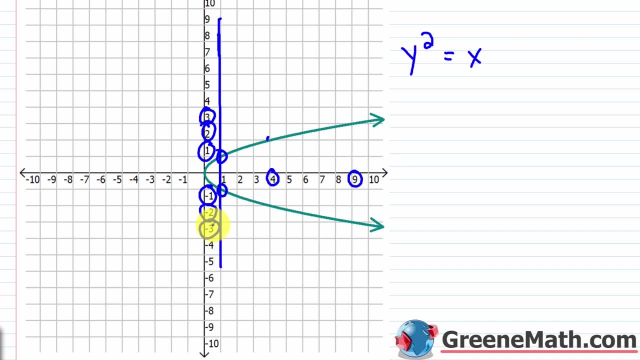 So this is not a function, because if I said, hey, what is the value of y, given that x is 9?? Well, you don't know whether to answer 3 or whether to answer negative 3. It could be either one. 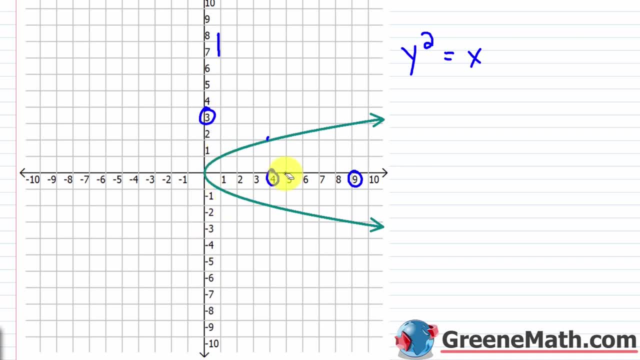 So not a function. Now I want to erase all this And I want to talk for a minute about the domain and range. What is the domain? Again, it's the set of x values. So what can x take on here? 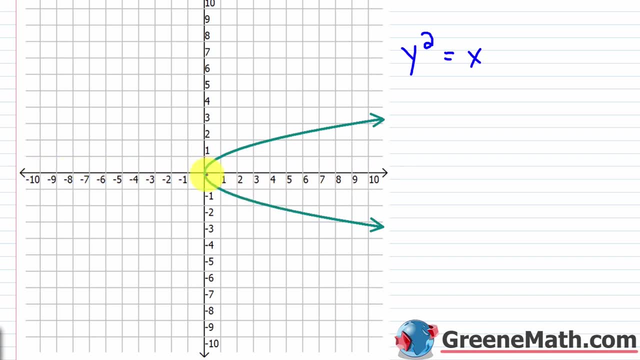 Well, if I look at the graph here again, this is the x-axis. Do you see any part of this graph that is to the left of 0? No, you do not. Why do you think that's the case? It's because, again, I'm using the squaring operation here. 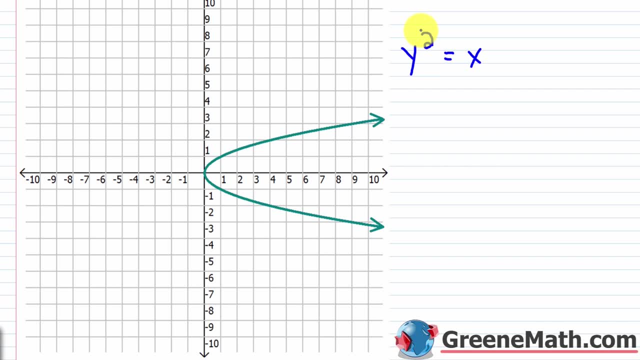 So if I square something, the result is going to be 0, or it's going to be positive, but it's never going to be negative. So that means that x can only be 0 or positive. So let me go back here and we'll write our domain. 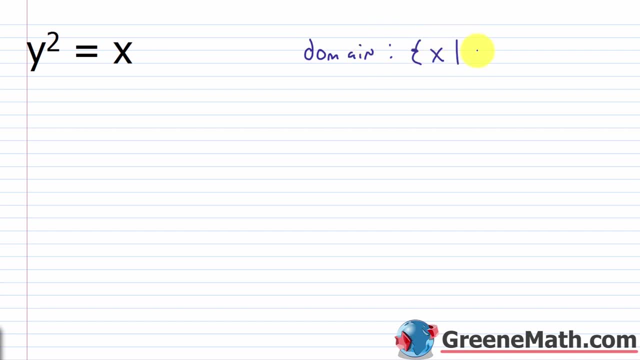 And we'll say that the domain is the set of all x values, such that x is greater than or equal to 0. And again, this is set builder notation, So the set of all x values. So if I'm thinking about values that I could choose for x, 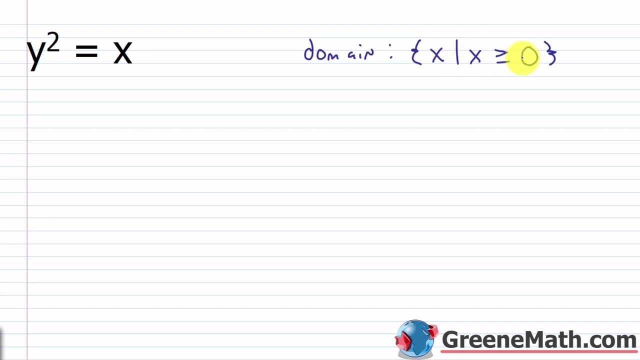 it's going to be such that the value of x is greater than or equal to 0. That's all we're saying In interval notation. you'd put a bracket next to 0, then comma infinity. Make sure you have that bracket, because 0 is included. 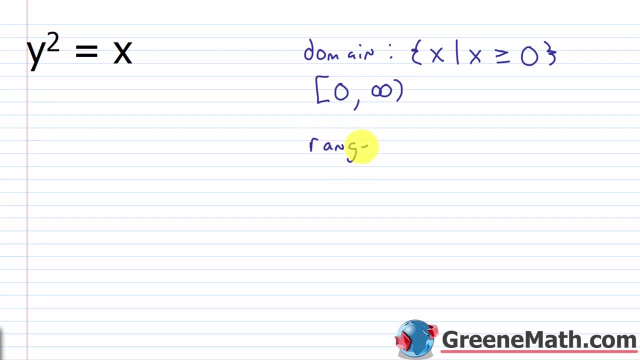 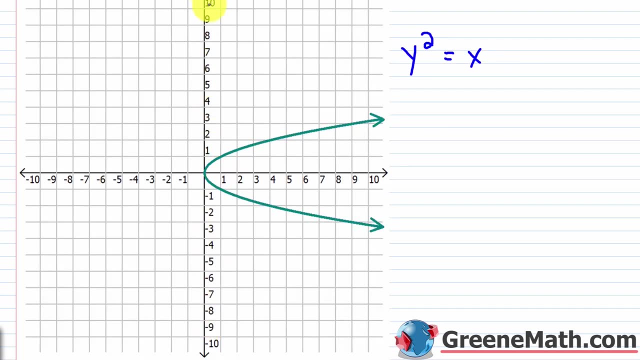 Now, as far as the range goes, When we think about our range, what would that be? Well, we go back to our graph. Think about the y values. now, This is the y values going up and down. Forget about the x values. 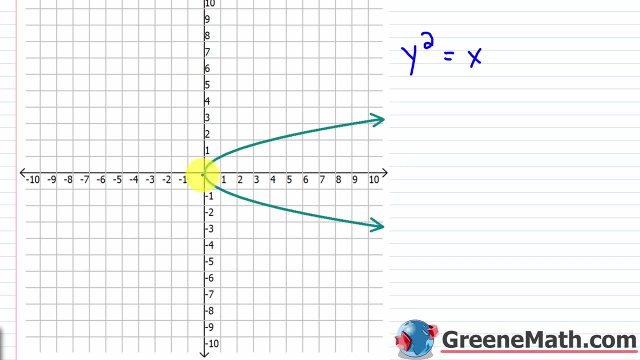 It's apparent that I have some that are negative, I have one that's 0, and I have some that are positive. So the arrows here indicate that this would continue going up forever and going down forever. So it looks like I can get any value for y that I want. 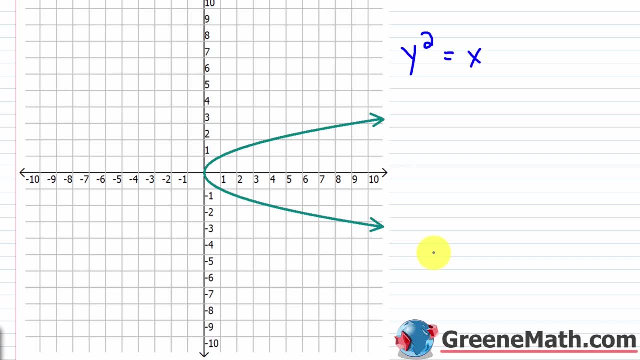 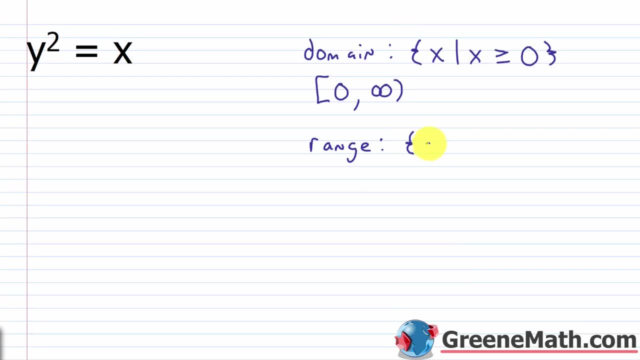 And yeah, if I'm taking something and squaring it, I could square a negative, I could square a 0.. I could square a positive. So there's no restriction on the range. The range can be whatever. So the range would be all real numbers. 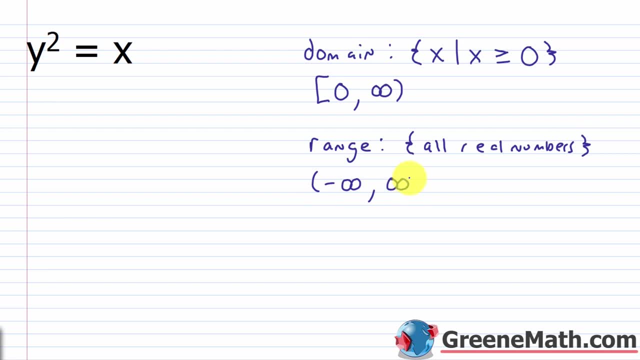 So that's from negative infinity to positive infinity, And another way to look at this. if you didn't want to waste your time to graph it, you said, hey, I don't want to do that, I just want to look at the equation. 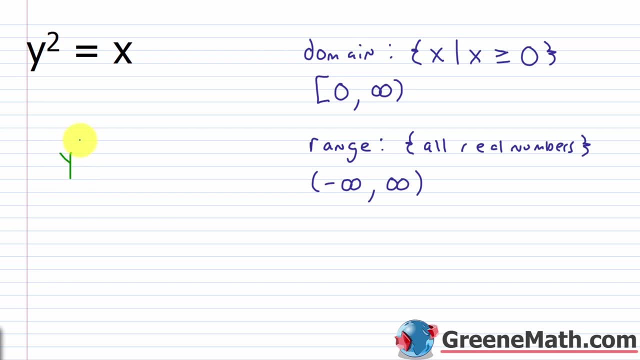 Well, you could solve this guy for y. So I have y squared equals x, And we talked about using the square root property in algebra 1.. For those of you that haven't taken algebra 1 yet, you're just kind of jumping in. 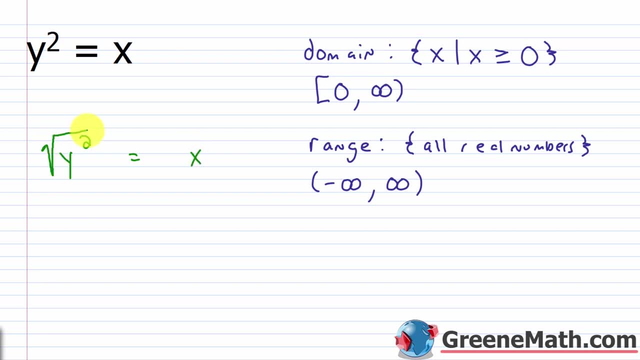 You don't know about the square root property. Basically, if I take the square root of this side, I've got to allow for the positive and the negative square root of this side. So what would happen is this: cancels with this and I have: y is equal to plus or minus the square root of x. 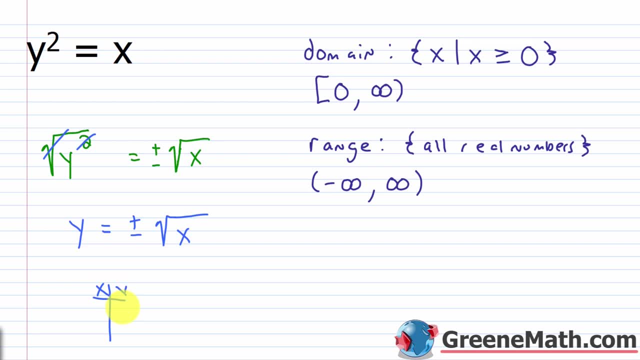 So, in other words, if I'm making a table of values, it would be completely obvious. It would be completely obvious that for each x there's more than one y, Because whatever I plug in here, once I take the square root, 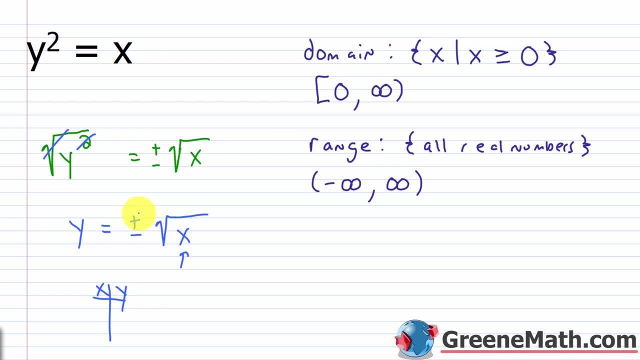 I've got a positive version and a negative version. The only exception to that is going to be 0. If I have 0, the square root of that is 0. There's no plus or minus 0. It's just 0.. 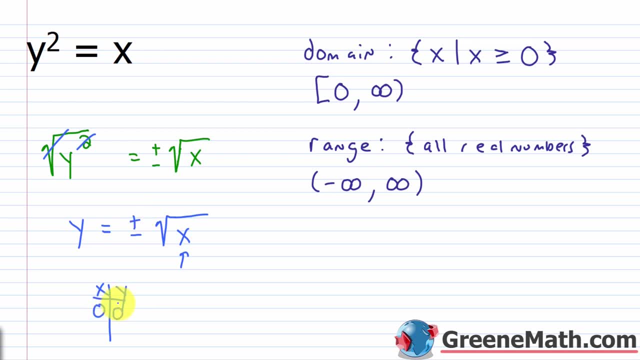 So if x is 0, y is 0. That makes sense. But for anything else, if I plug in a 1 for x, I know y would be positive and negative 1.. Square root of 1 is 1.. 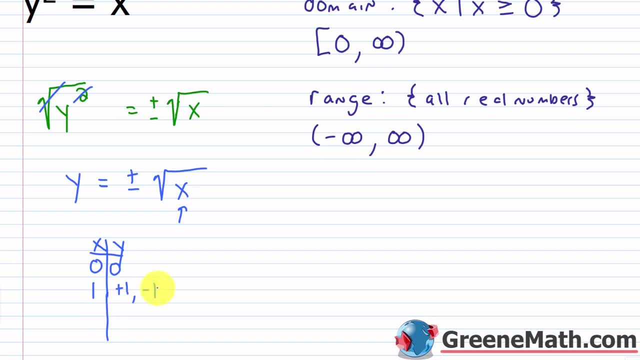 You'd have plus or minus 1.. And then minus 1.. So right there, it fails the definition of a function. If I use something like 4, square root of 4 is 2.. So you'd have plus or minus 2.. 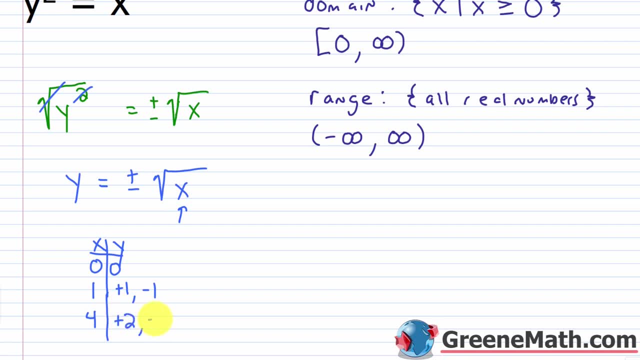 So if x is 4, y is plus 2 or minus 2.. As one that's not so clean, let me kind of scooch this up a little bit. I can even use 5.. Let's say x is 5.. 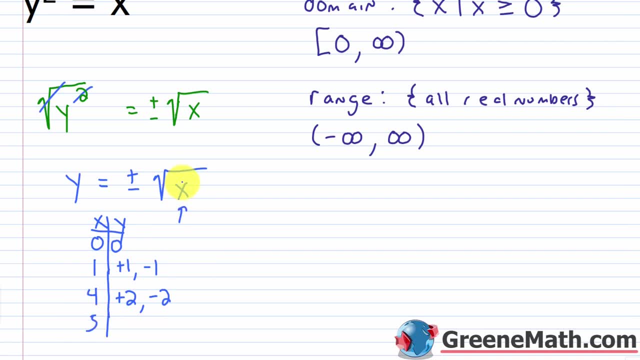 Plug in a 5 there, I'm going to have the square root of 5.. That's not a rational number, So what I would just do is I'm going to plug in a 5.. I would just do is list it as a square root of 5.. 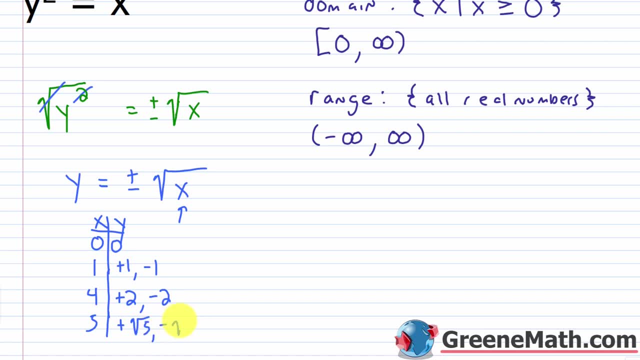 So I could say this is plus square root of 5 and minus the square root of 5.. But you get the idea of why this isn't a function. That's the main thing here. It's just a simple fact that if I have at least one x value, that 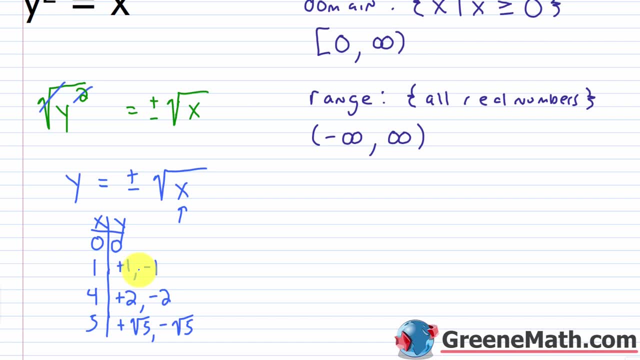 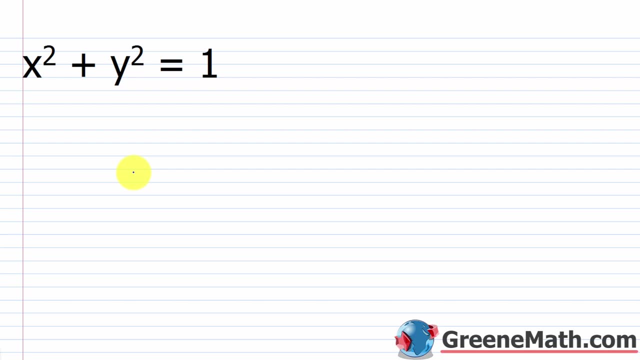 is linked to or corresponds to more than one y value. I do not have a function, Let's take a look at another one. So here we have: x squared plus y squared equals 1.. Those of you that have taken geometry or trigonometry: 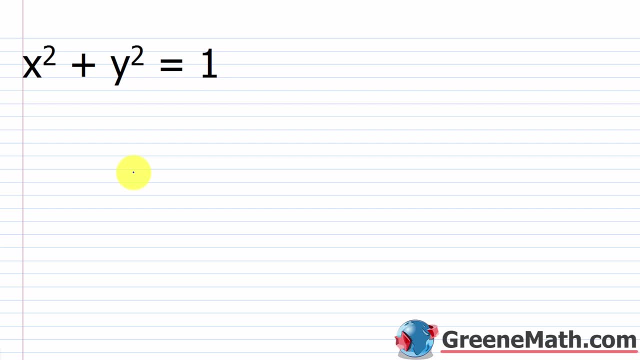 you know this is the unit circle, So is this a function? Is a circle going to be a function? No, Think about it. A circle looks like this. I know that's not a good drawing, but if I draw vertical lines through that, 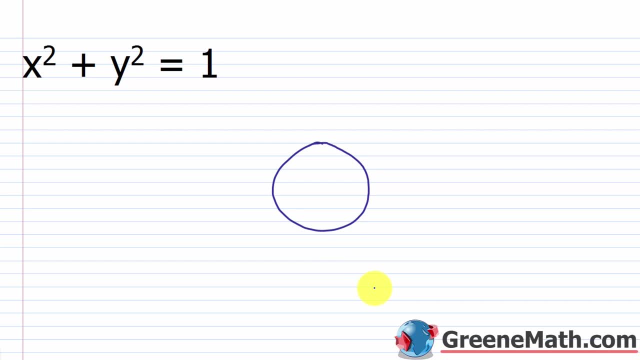 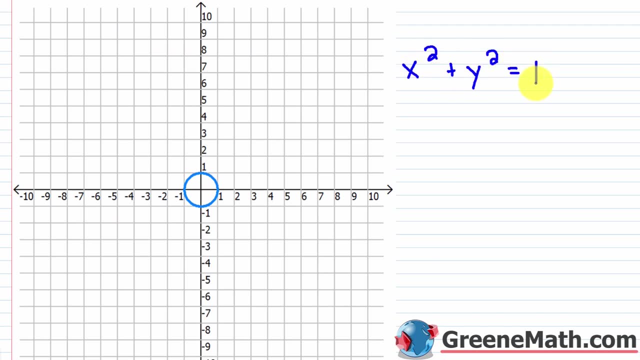 it's not going to make it. It's going to impact that graph in more than one location. But let's go ahead and look at the graph. So this is: x squared plus y squared equals 1.. Again, if I draw vertical lines here, 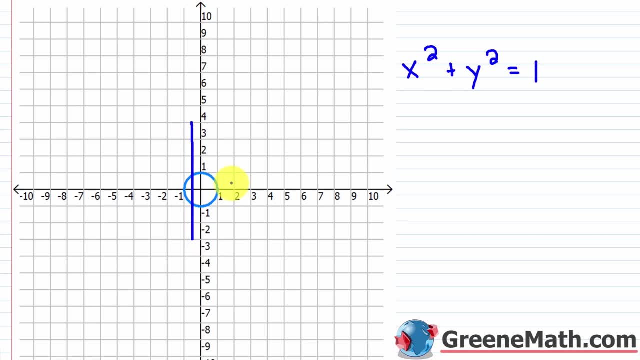 let's just draw two, because it's such a small kind of graph. you can clearly see this. This violates the definition of a function. My vertical line hits here and here. My vertical line hits here and here, So this is not a function. 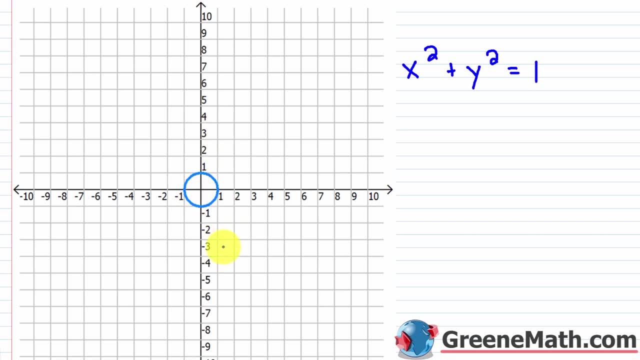 Now, when we start talking about the domain here, you're going to really be pressed on this one. I'm going to go back and look at the equation and explain why. But if you look at the domain, look at the x values, this thing can take on. 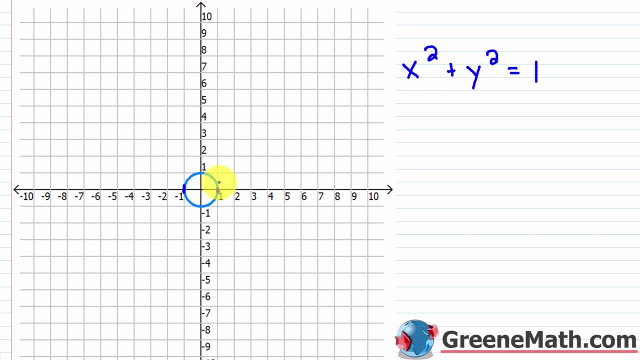 Starting at negative 1 and including negative 1 up to positive 1.. Look at the range Starting at negative 1 down here up to and including 1.. So we seem pretty limited. Why is that the case? Let's look at the equation. 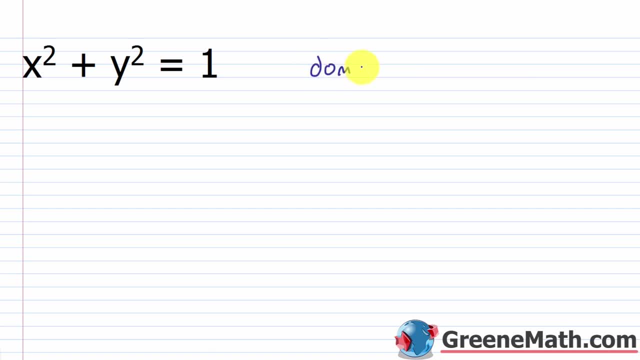 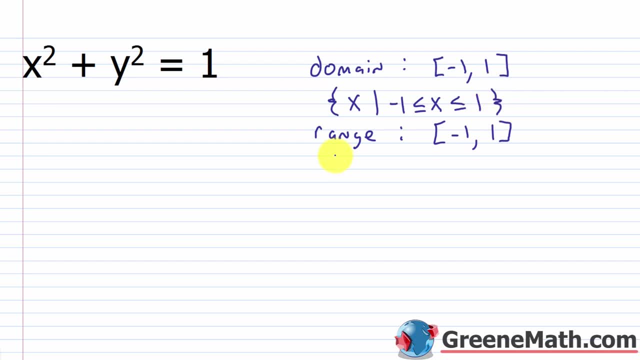 And less than or equal to 1.. You could write it like that, Or for this one you could say: the set of all y, such that Same thing, Negative 1 is less than or equal to y, which is less than or equal to 1.. 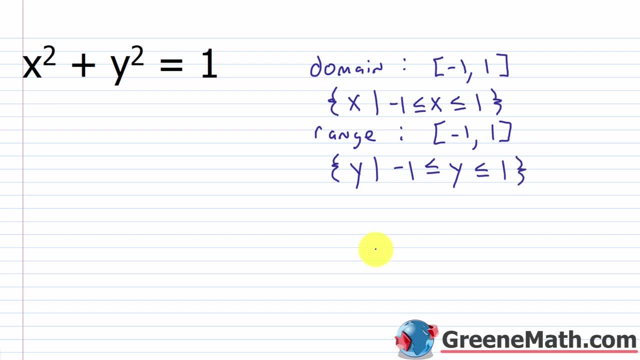 So two kind of different ways to write that, A bunch of ways to write it. Write it however you please. With this one, I want to solve it for y real quick. So we have x squared plus y squared equals 1. Move x squared over here. 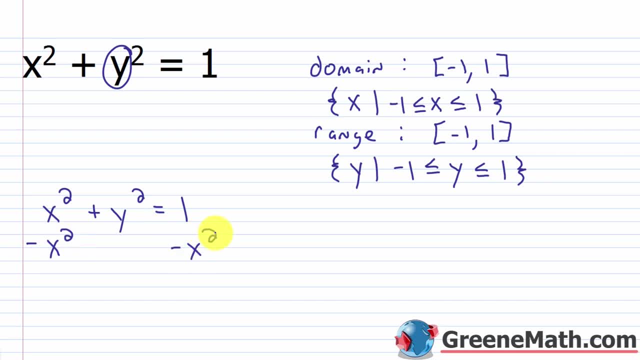 So let's subtract x squared away from each side of the equation equation, and I'm just going to erase it. So we'll have: y squared is equal to negative, x squared plus 1.. So y squared is equal to negative, x squared plus 1.. Okay, how do I? 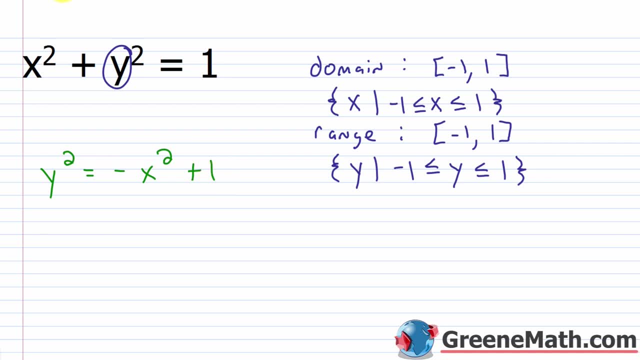 get y by itself. Take the square root of both sides. Again, if I take the square root of this side, I've got to go plus or minus the square root of this side. okay, So I'll go plus or minus the square root of this side. So that means that y is equal to plus or minus. 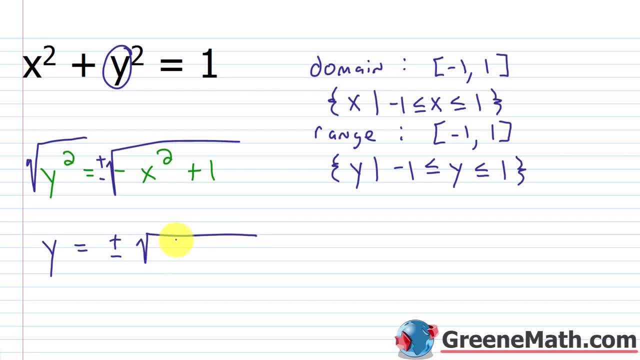 the square root of negative x squared plus 1.. I'm just going to flip the order there and I'm going to write 1 minus x squared. So looking at what's inside that square root symbol, we should see something. Something should jump out, as it explains why the domain 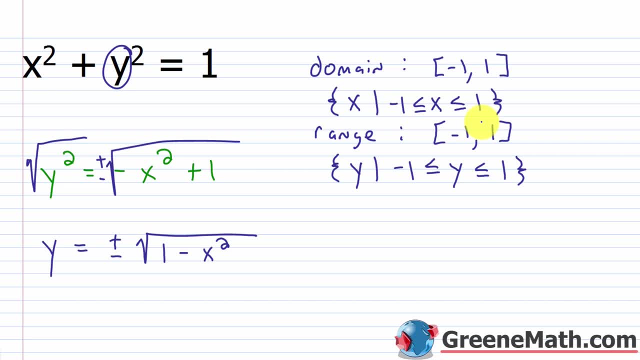 and range is so limited. The first thing is: can I take the square root of a negative number? Can I have square root of negative 5?? No, that is not a real number. The answer to that is yes, but only with the correct answer. 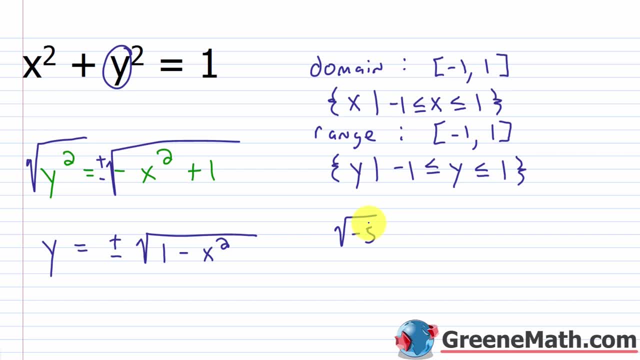 It's a complex number system. So if you've worked with imaginary numbers in the past, you're probably screaming right now like, yeah, we can do it, You use i blah, blah, blah. Okay, we are only working with real numbers. So with the real number system, the 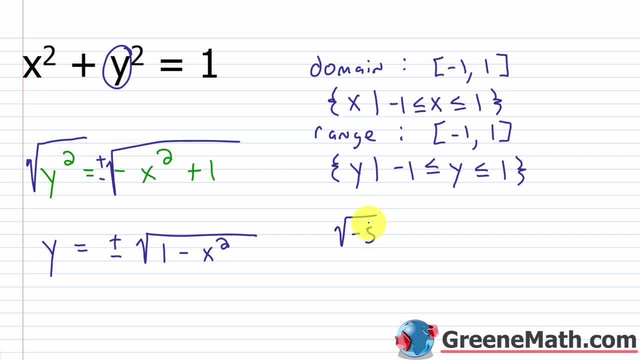 answer to that is no. There is no number that results from the square root of negative 5. It does not exist, okay, in the real number system. So what that means is that the result of this has to be 0 or positive. It cannot be negative. Now look at what you're starting. 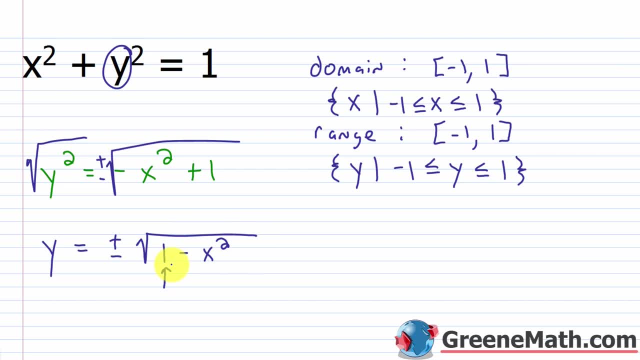 with. Imagine I start with a dollar in my pocket. okay, What can I spend without going into debt? without using credit cards, I can spend $1,. okay, I can spend less than a dollar, but the most I can spend is a dollar. So the most that x can be is 1, because I'm going. 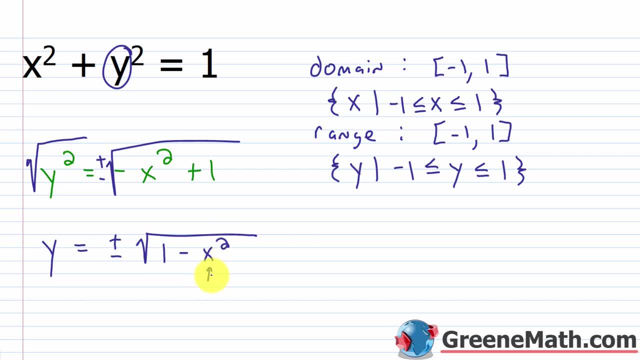 to take something and square it. If it's anything between 0 and 1, I'm okay. Anything larger than 1, let's say 2, for example, 2 squared is 4.. 1 minus 4 is negative 3.. 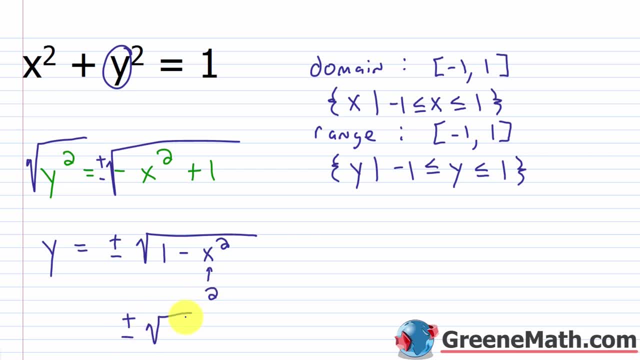 The square root of negative 3, if I had plus or minus the square root of negative 3, I can't do that using real numbers, So that's nonsense, I can't use that. okay, So the most this can be is going to be 1.. 1 works. 1 minus 1 would be 0. That's okay. Anything between: 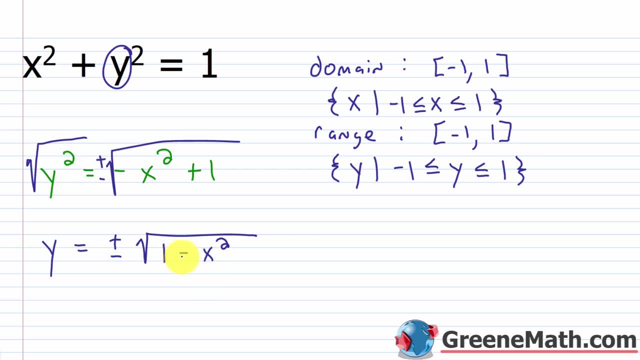 0 and 1, including both, works. If I have 0 there, I'd have 1 minus 0, that's 1, square root of 1 is 1.. That's okay, And then going down into the negative values, I know that. 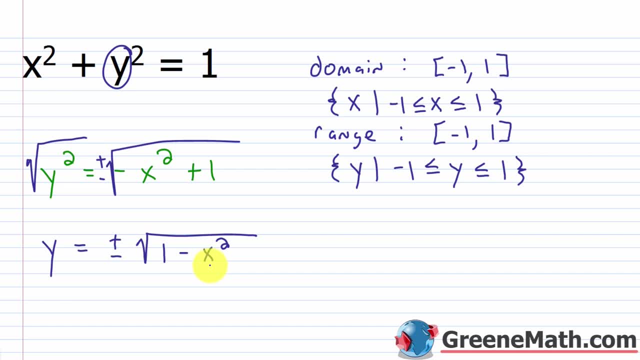 I can go as far as negative one. anything past. that's going to be a problem because again, even though I'm squaring something, I'm subtracting it away. if I said one minus negative two squared negative two squared is four, I've got the same problem. I've got one minus four, that's negative three. so the most that. 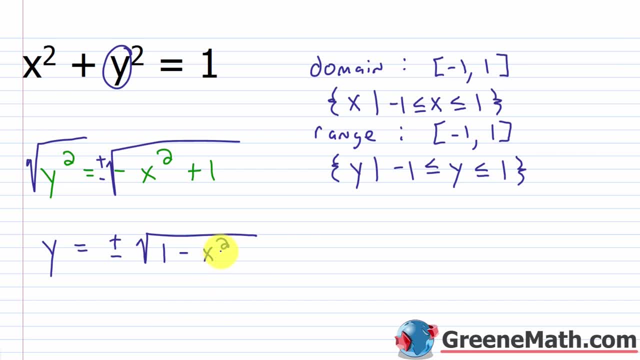 x can be is one. the least it can be is negative one. so it's got to be from negative one up to including one. and what would that produce? well, the same thing in y if, on the high side, I produce one. well, the square root of one is one. I'm going to have plus or minus this one, so I have positive one. 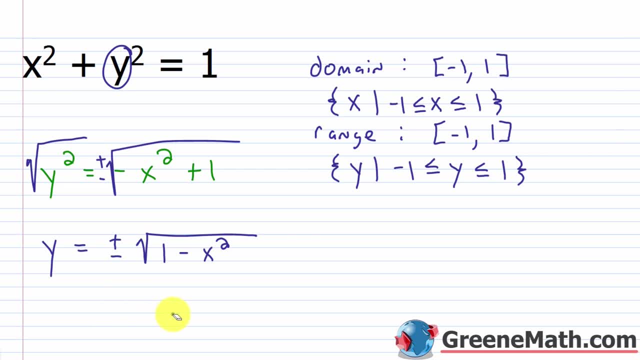 and I have negative one. so that's where you get this domain and range. from the inputs, the x can be as low as negative, one as high as one. the range- the output, can be as low as negative one or as high as one as well. so that's why this is the unit circle. this is not a function and your domain. 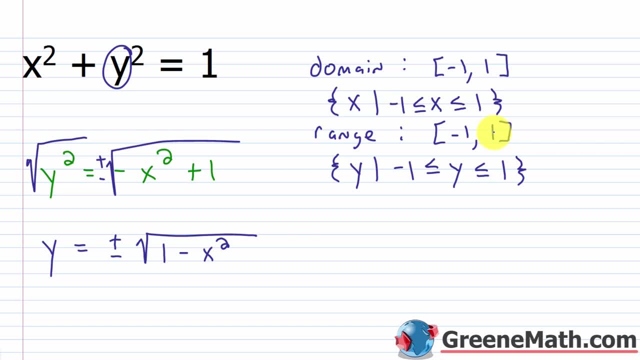 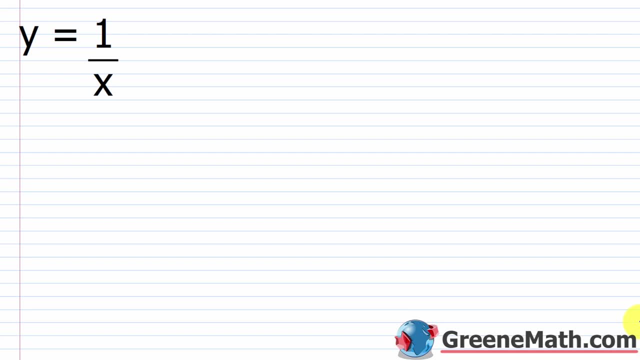 and range are both limited, from negative one up to and including one. all right, for the next one we're going to look at y. y equals one over x. so obviously, before we jump into this thing, we all know that we cannot divide by zero, so we can't have an x value of zero. so we know our domain will be limited to that. 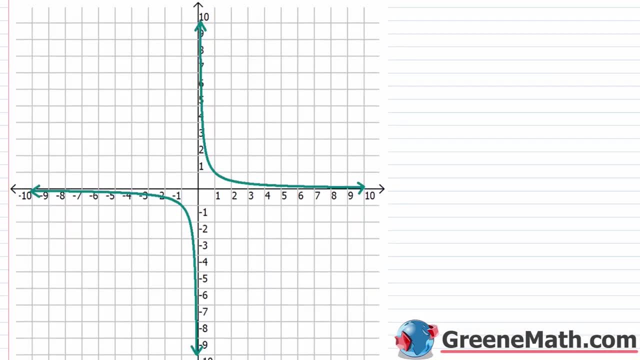 so I want to look at the graph of this. so we have y equals one over x, as we expect when we have an x value of zero. I want you to notice something: we get very, very close as we go this way towards zero. we get very, very close to having an x value that zero, but we will never have an actual x value that. 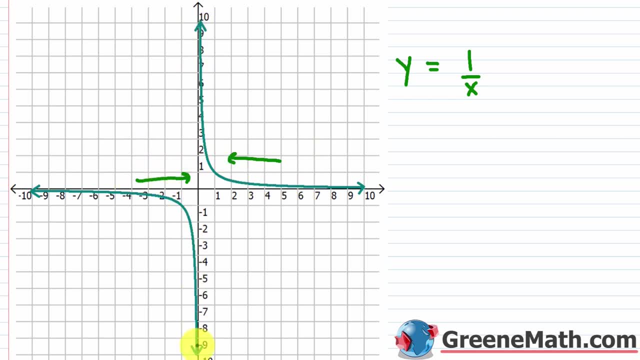 zero. not this way and not coming from this way as well. we have something known as an asymptote here. so if I drew a vertical line that was the same as the y-axis, let's just say I draw a vertical line here, and I know that's not precise, but let's just say it is so at x equals zero. 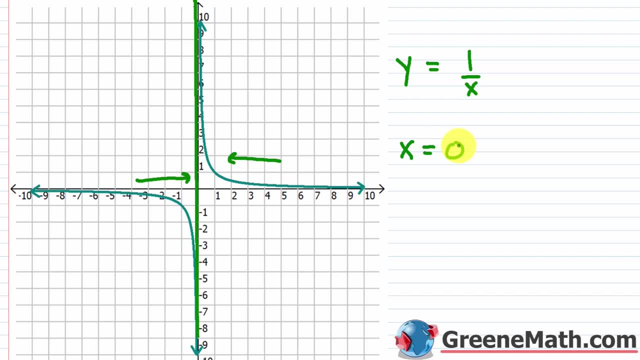 we have something known as an asymptote, so that line that exists at x equals zero. my graph will approach it, it'll get very, very close to it, but it will never, ever, ever touch it. now let's explore why we have this phenomenon. for a second, well, we can think about dividing by really, really small. 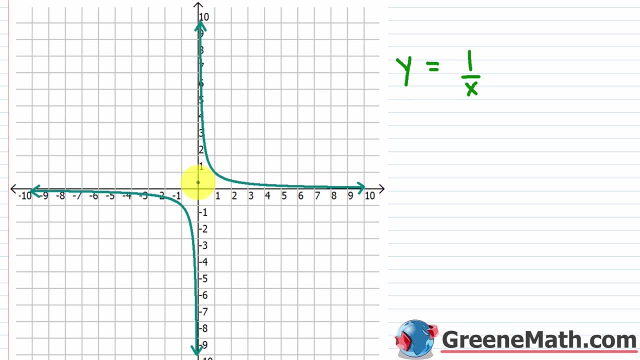 numbers that are close to zero, but not quite zero, as I divide one by something close to zero. what happens is it becomes a zero, and then we have a line that exists at x equals zero, and we have a line that exists at x equals zero, and then we have a line that exists at x equals zero, and we have 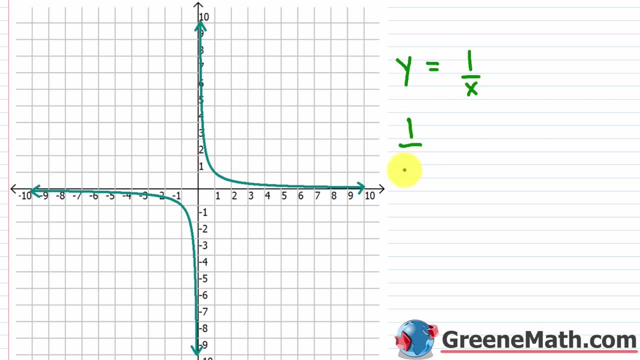 larger and larger. so if I take one and I divide it by 0.5, this is going to give me two. if I take one and I divide it by something closer to zero, let's say 0.25- this is going to give me four. 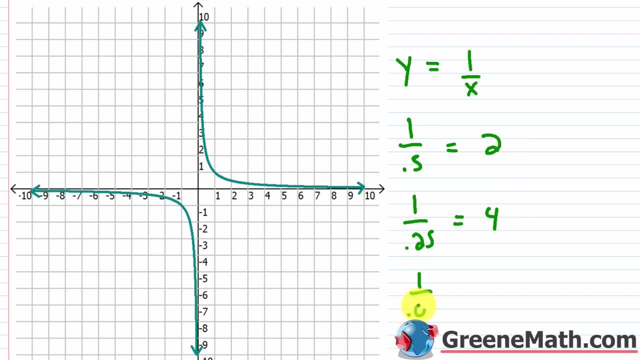 notice how this increased. if I take one and I divide it by 0.05, this would give me 20 right. so on and so forth. so the closer I get this denominator to zero going this way, the bigger the number is going to go. so you see how this kind of hockey sticks up. so 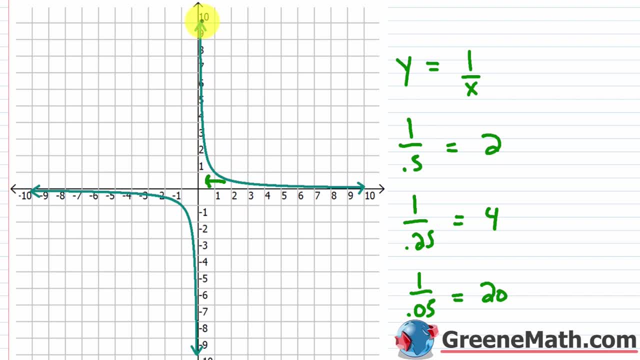 The closer I get an x value to zero, the larger y is going to get, And I can make it infinitely large as I get infinitely close to an x value of zero. So that's why this guy right here would approach an x value of zero. 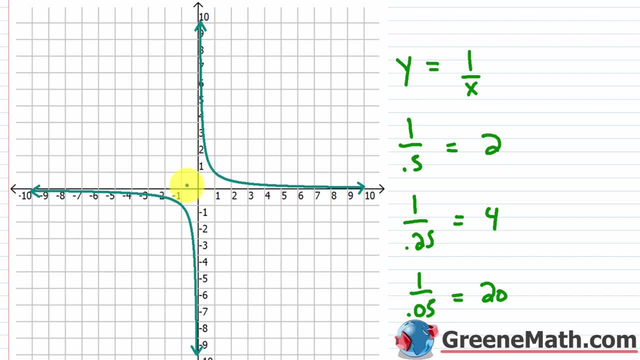 but it would never, ever actually give me one. Okay, so the same phenomenon happens when we think about the negative direction. If I'm coming from here going this way, coming from the left going to the right, this graph will approach an x value of zero, but it will never, ever, ever give me one. 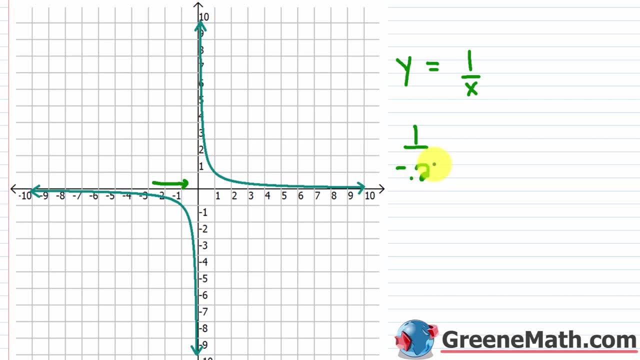 If I'm dividing one by negative 0.25, this is negative four. right, I'm just getting a bigger negative number. One divided by Negative 0.05 is negative 20, right, So on and so forth, So I can make this value infinitely large. 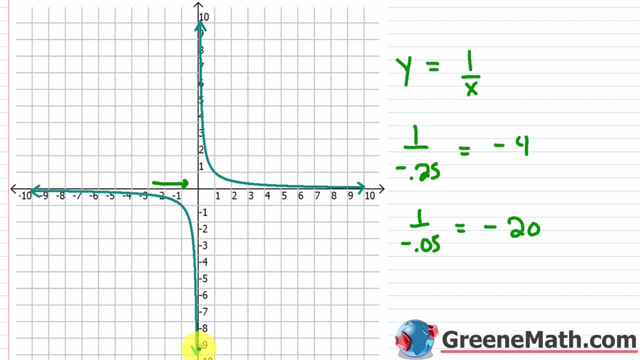 or we can think about it as a bigger and bigger and bigger negative by just making this number as close to zero coming from the negative direction. So you'd have like negative 0.0000000000003, for example. Something like that would produce a very, very, very big negative number. 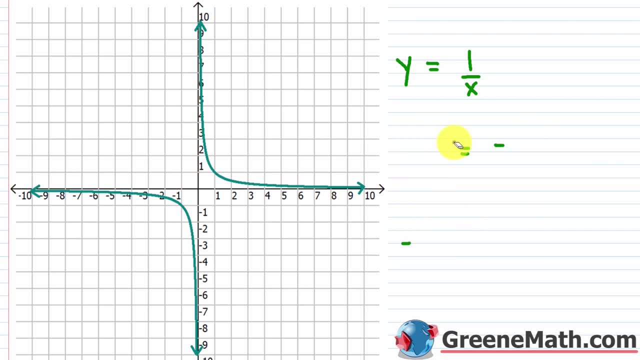 All right. So as long as we understand what's going on there, let's think about our domain and our range. Graphically we can look at it and it looks like the domain when we look at the x-axis. here can be anything negative. 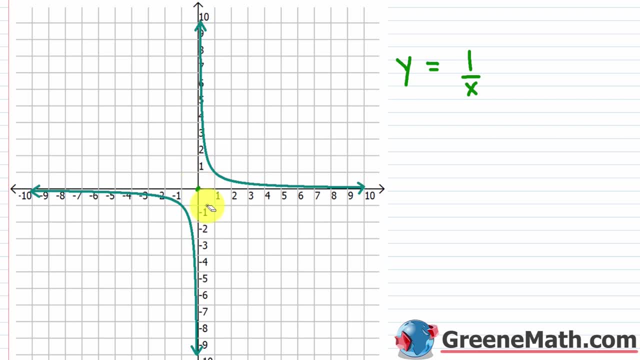 can be anything positive, it just can't be zero. What about the range? Well, again it looks like the same thing. It can be anything positive, it can be anything negative, but it can't be zero. So you can say you have another asymptote that occurs. 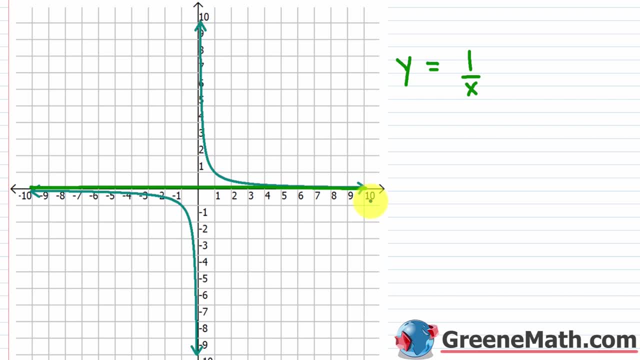 where y equals zero right, or the x-axis, where y equals zero. The graph is going to approach a y value of zero, but it's never going to actually give you one, okay, So it's going to get infinitely larger and larger and larger in terms of an x value here. 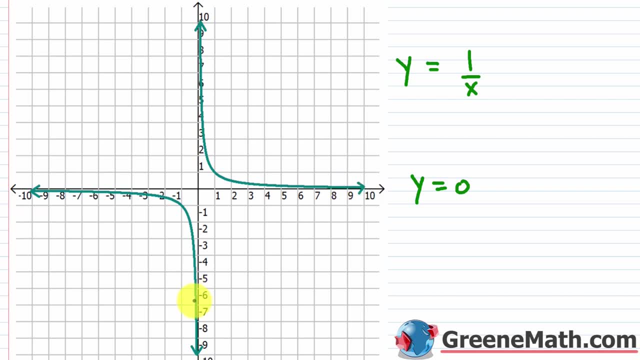 as y approaches zero, but it's never going to give you one. And it's the same thing here. As our y value approaches zero, the x value here becomes infinitely negative. okay, But the y value would never be zero as well. 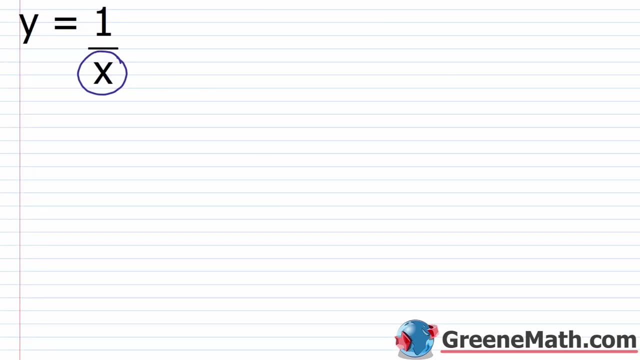 So when we go back and write our domain and range, we could say that our domain is the set of all x, such that x does not equal zero. We could say our range is the set of all y, such that y does not equal zero. 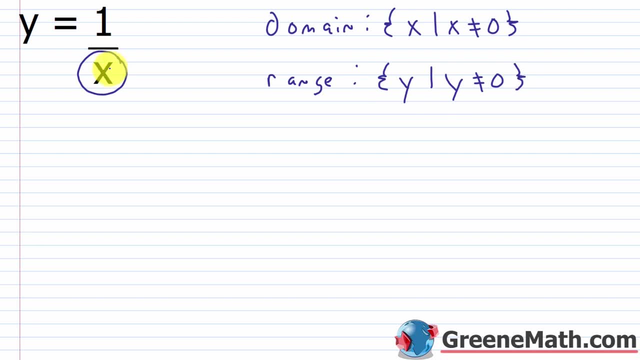 Now most people understand why x can't be zero. You can't divide by zero, That's obvious. Why do you think y can't be zero? We'll do a little bit of algebra, Multiply both sides by x and you'll make it obvious why. 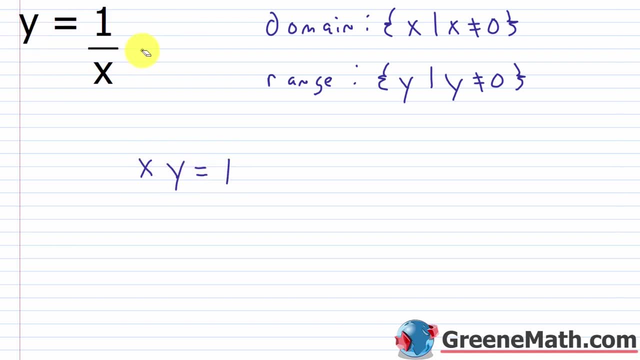 xy equals 1.. Think about that for a second. How can two numbers being multiplied together produce 1?? Well, you're multiplicative inverse property. It means they're reciprocals, right? So if I had 5 times 1, fifth, that's 1.. 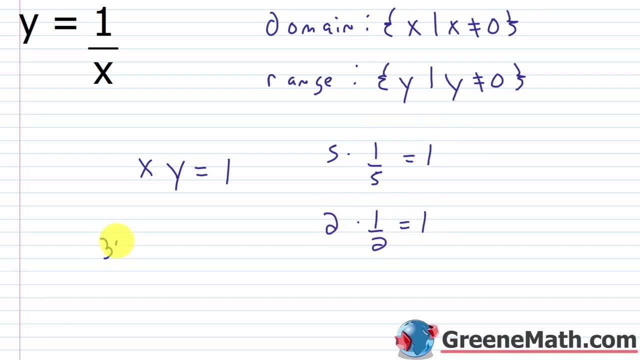 If I had 2 times 1, half, that's 1.. If I had 30 times 1, over 30, that's 1.. So these two values have to be reciprocals. Now, does zero have a reciprocal? 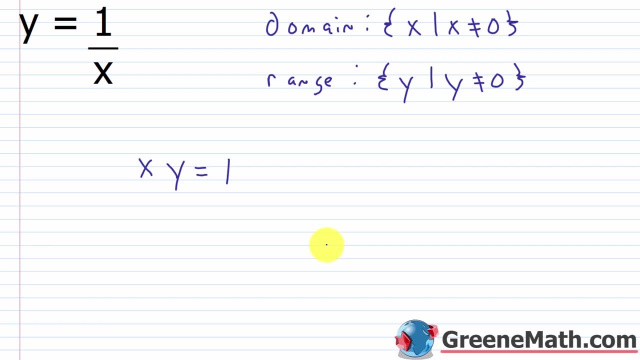 No Zero times. any number is zero, okay. So if x was zero y, no matter what it was, when I multiply them together, I'd get zero equals 1.. That's false. Same thing goes for y. If I plugged in a zero for y, no matter what x is, doesn't matter, I'm going to get zero. 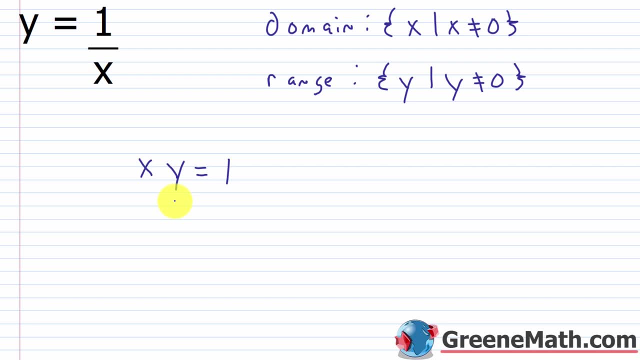 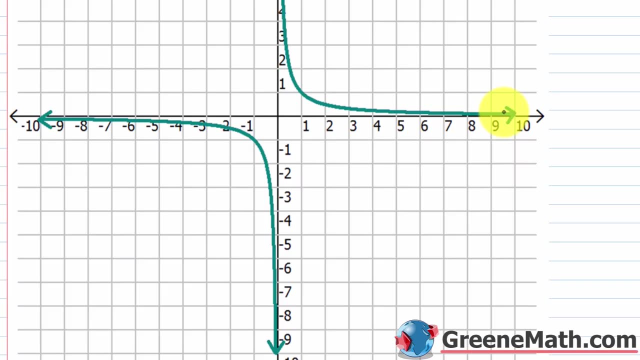 equals 1.. That's false. So my domain can be anything other than 0, as well as my range, So that can also be anything other than 0.. So, if I think about, is this a function or not? if I draw vertical lines, 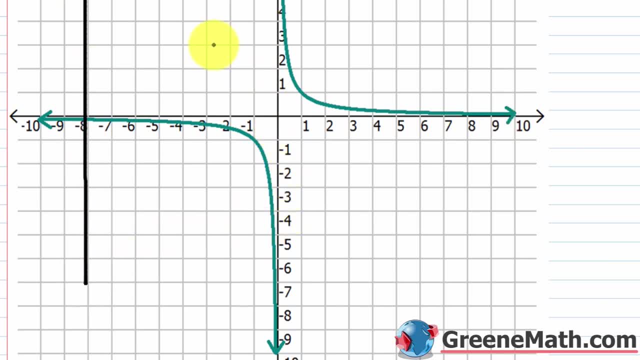 So those aren't perfect, but you can see in each case that the vertical line only impacts the graph once. So here it's obvious, here it's obvious, here it's obvious. This one is where it starts. 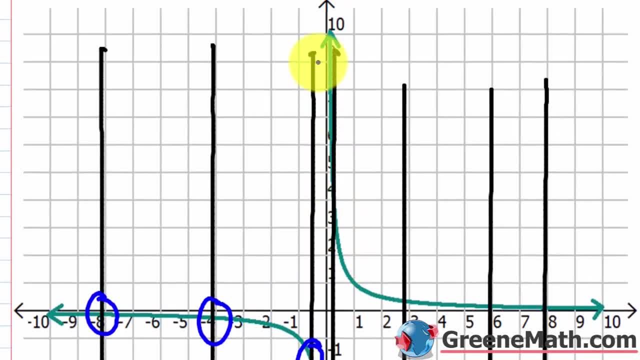 getting tricky because it runs into something that's going very vertical, okay. So it looks like, yeah, it's hitting more than once, but it's actually not The point of intersection, would be something like that. okay, I don't know what it actually is, but it would be something like that. 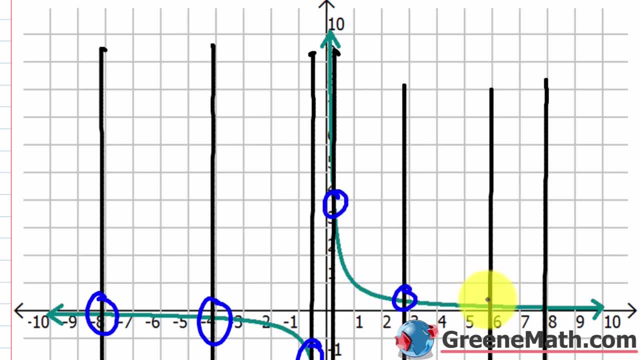 It would hit only once For every x. here you're just going to get one and only one y. So these are kind of tricky to use the vertical line test on. but if you plug in something for x, you'll get one y. Now you would say that this function is only defined when x does not equal zero. okay, x cannot. 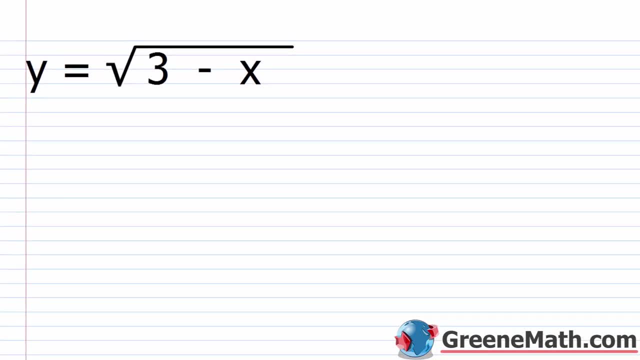 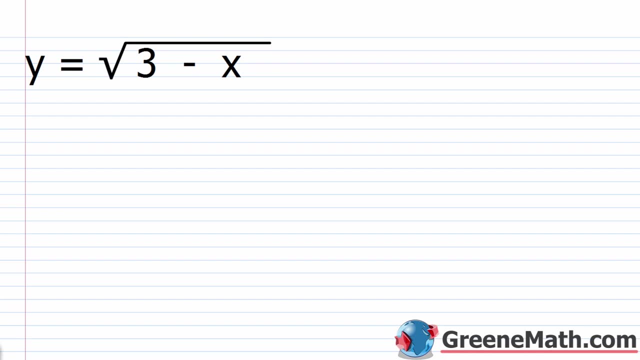 equal zero. y cannot equal zero, All right, so let's take a look at one final one. So I have here that y equals the square root of three minus x. So let's take a look at the graph. So we look at: 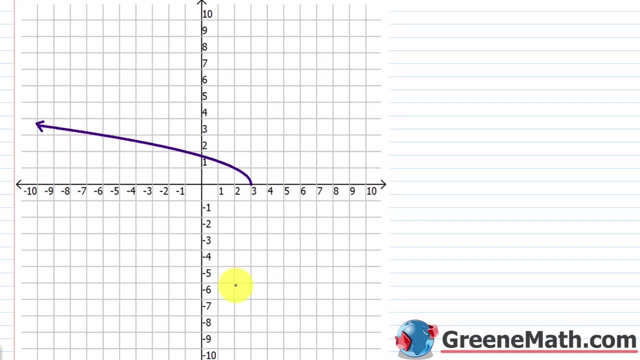 this one, and it's very easy to see that it is a function. Now it starts here at three, in terms of the x value, and it goes to the left. I don't see anything to the right and I'm going to explain. 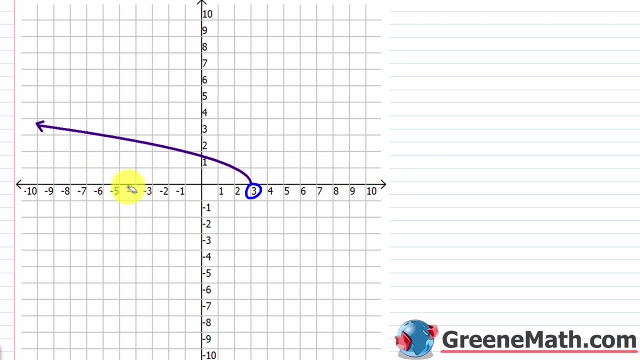 why in a second, But I want to draw some vertical lines here just for the sake of completeness. It's pretty obvious that this one is a function. Won't get any arguments on this Now. this function is defined for values of x that are three or less. 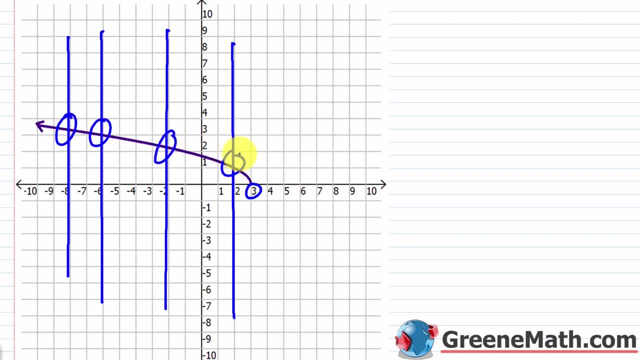 So this, this, this, this, every vertical line I would draw would only impact the graph in one location. Now my observation for x is that, again, x is three or less. What about my observation for y? Do you see any y values down here below zero? No, You see zero. and then this increases. 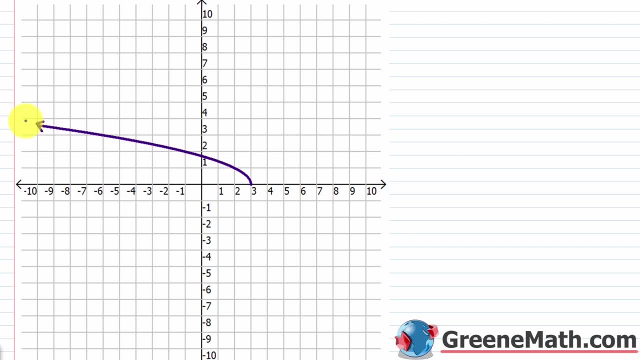 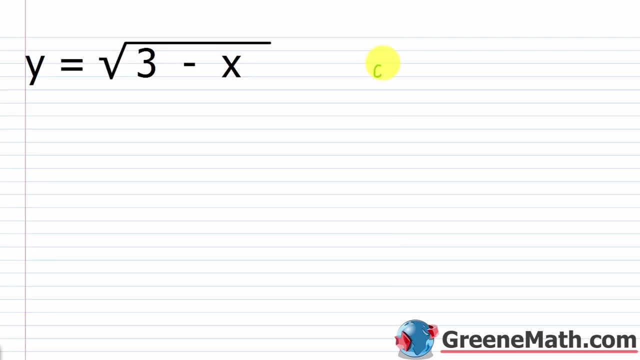 and this is an arrow drawn, so we know this would increase forever and ever and ever. So y could basically be zero or anything larger. So let's go back and let's list our domain and our range And let's think about why this is the case again. So I 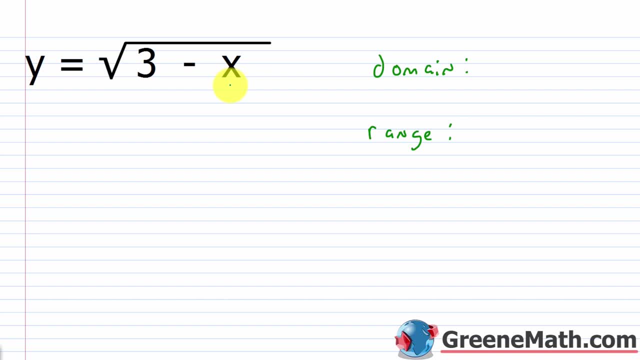 have the square root of three minus x. Again, this square root thing. I don't want to take the square root of a negative number. So if I'm starting with $3 in my wallet, what's the most that I can spend without going into debt? $3.. So that's why x can be at most three. So the domain: 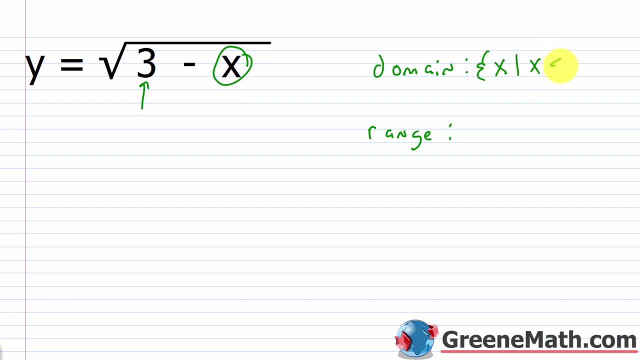 would be the set of values of x and the set of values of y and the set of values of y and the set of all x, such that x is less than or equal to three. Now, in this particular case, could x be? 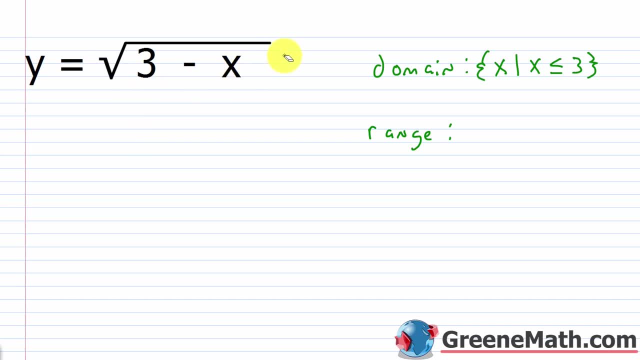 negative? Yes, it can, And the reason for that is because I don't have any squaring operation or anything crazy like that. If I subtract away a negative, I'm adding a positive. So if I had the square root of three minus, let's say negative six as an example, well, that would be the square. 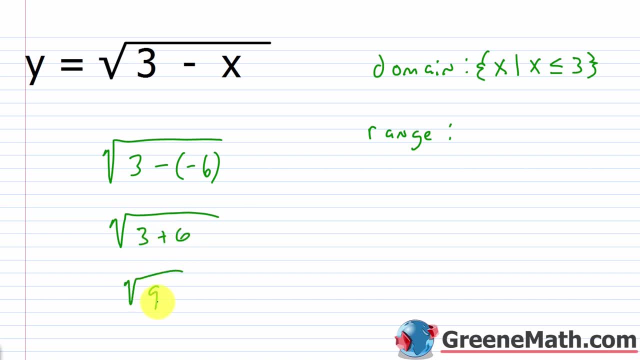 root of three plus six, which is the square root of nine. Okay, square root of nine is three. So I know that I can have any negative value that I want. That would be okay, And I can have zero if I want. Three minus zero is three. No problem there. I can have any positive value I want, up to 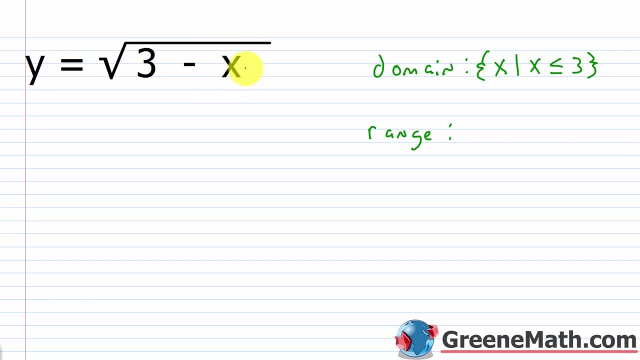 and including the number three, If I have a three here. three minus three is zero. The square root of zero is zero. Now, one thing you would notice is that there's no plus or minus out in front. This is just the principal square root of three minus x. So we're okay there. That's fine Now. 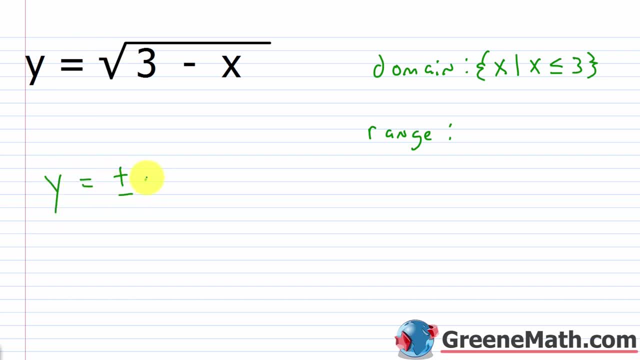 if I saw something like: y equals plus or minus the square root of three minus x. that's a problem, Because when I get a result here, I'm going to have the positive and the negative. So for each x I'm not going to. 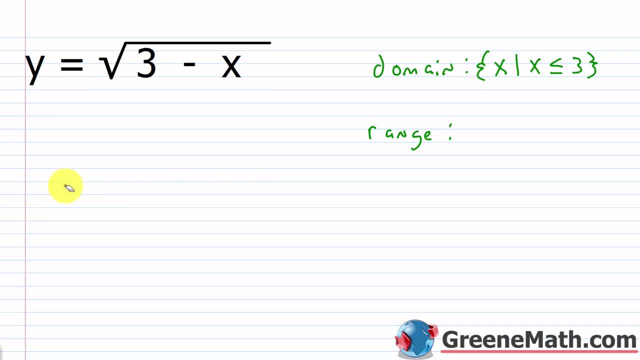 just have one y, So that would be an issue. But in this particular case, we do have a function. Now my range is what? Well, we know that the least it can be is zero. We saw that with the graph. And why is that the case? Well, the most I can make this is three. So three minus three is 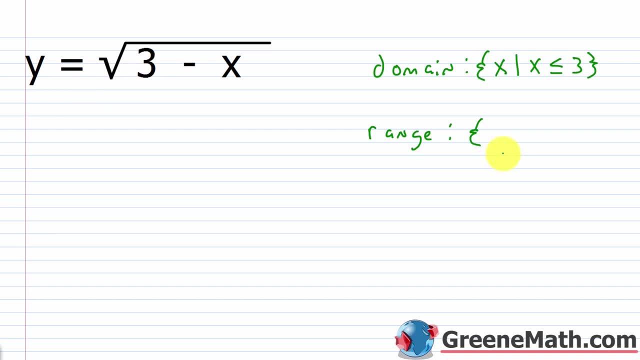 zero. So that's where y is zero, And then I can make this grow or have a higher y value by choosing a lower x value, because I'm subtracting less away And when I get into negatives I could choose negative one million and I could make y really, really, really big. So really y can be anything. 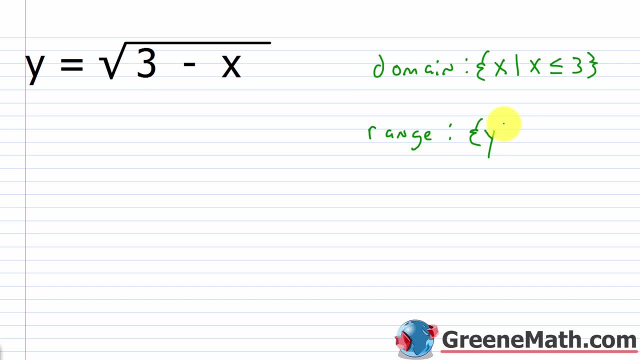 that's zero or larger, So the set of all y, such that y is greater than or equal to zero. And of course you could write these in interval notation. You could say the domain is from negative infinity up to and including three And the range is from zero out to infinity. 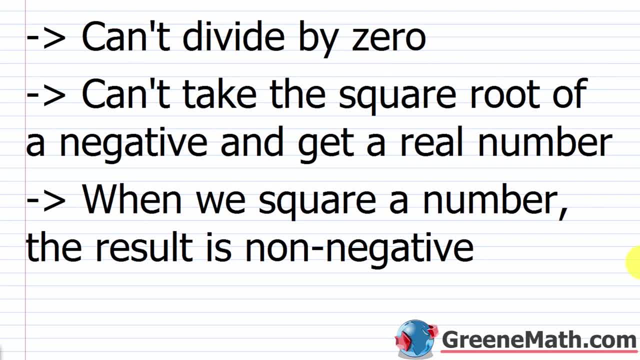 All right. So let's just kind of wrap this up with some key points here. So when you're looking for the domain and the range, remember you can't divide by zero, You can't take the square root of a negative and get a real number, And when we square a number, the result is non-negative. 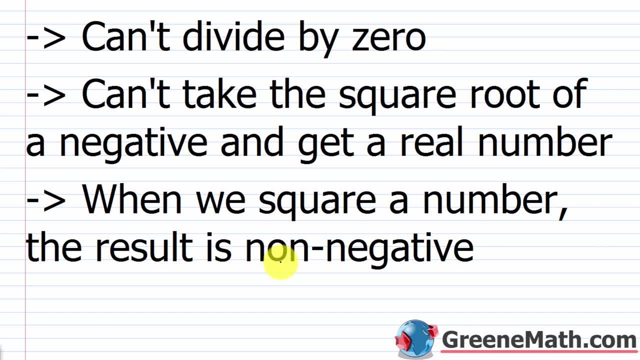 So if you write down those three things, it's really going to help you when you start getting challenged on these questions. Look for again: can't divide by zero, can't take the square root of a negative, And when you square something it's going to be non-negative. Hello and welcome to Algebra 2, Lesson 23.. 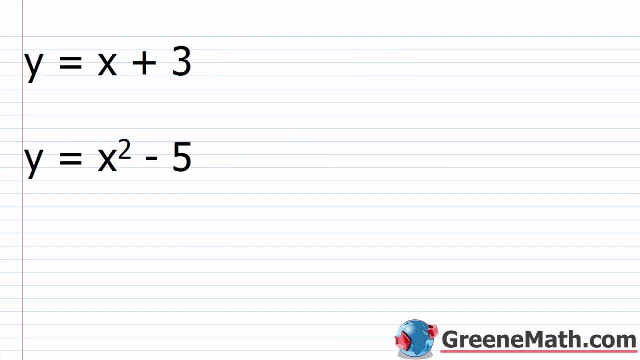 In this video we're going to learn about function notation. All right, So we're going to start by looking at two brief examples here. We have y equals x plus 3, and we have y equals x squared minus 5.. So at this point we know that these two relations are functions. I input something in for. 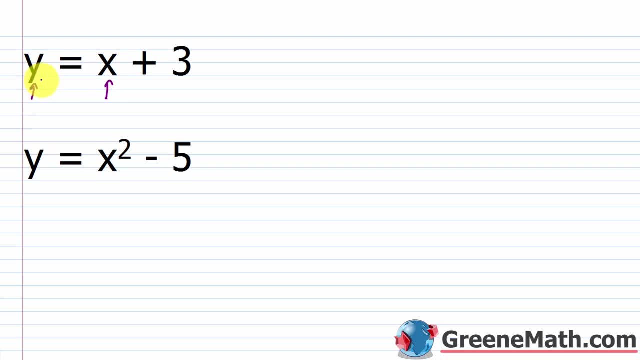 x, I get a unique output for y. So, as an example, let's say I plug in a 5 for x. 5 plus 3 would give me 8.. So my output for y is 8.. As I change the value of x, I'm going to change the value of y. 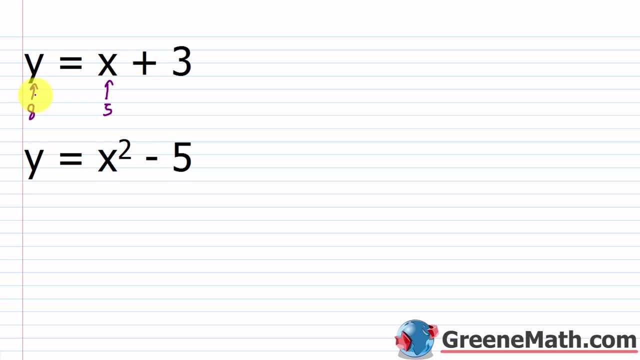 So y depends on my input for x. So again, x is the independent variable, Y is the dependent variable. It's the same with this example here as well. If I plug in, let's say, a, 2 for x squared is 4.. 4 minus 5 is negative 1. If I change the input for x, I change the output for y, So y. 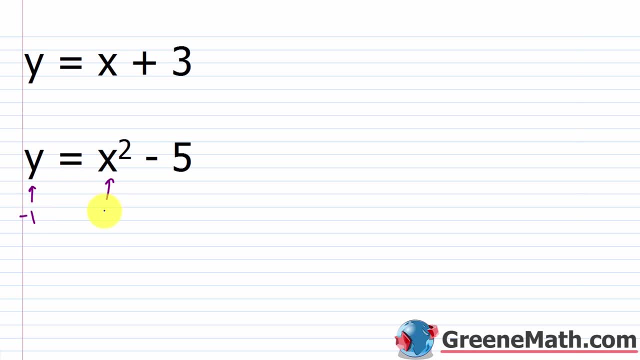 depends on x. If I say, made this 3,, 3 squared would be 9.. 9 minus 5 would give me 4.. So as I change my independent variable x, my dependent variable y is going to change Now when we start. 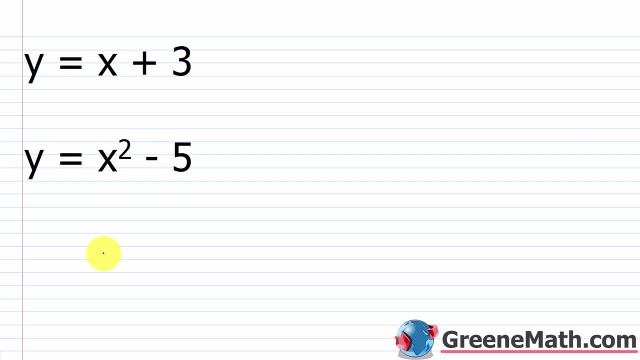 talking about functions generally, we start out with the typical y equals something. As we move on, we're going to replace that notation of y equals something with f of x equals something And let me tell you this is a very big cause of confusion. A lot of students. 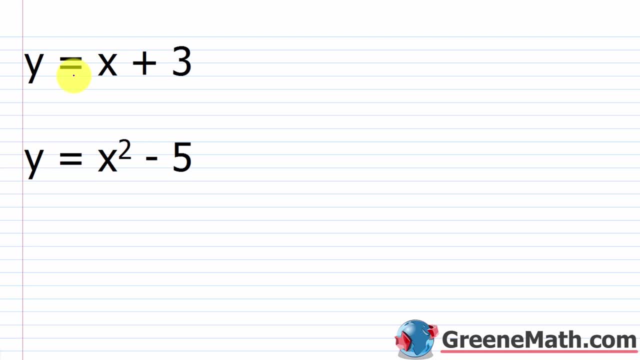 are like: where did y go? Bring y back, Why can't I have y anymore? It's gone and it's not going to come back. So as you get into higher math, particularly college algebra, they're not going to spend any time explaining that y is the same thing as f of x. They're just going to present it. 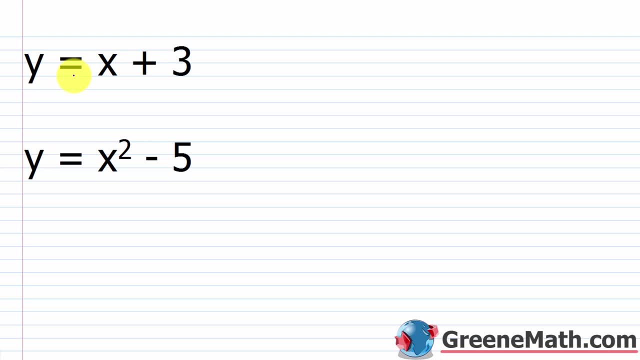 and you're going to have to do the same thing over and over again. So you're going to have to move on with it. So I want to take the time here to make sure you understand this. Functions are generally named with f, g or h, So you'll see f, g or h And it might be lowercase, it might be. 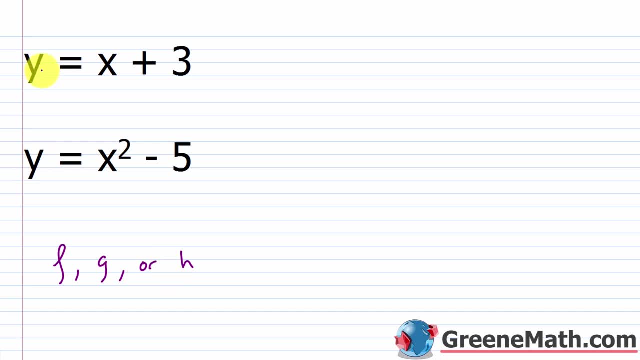 uppercase whatever they want to use And typically what you're going to see is, let's say, I'm naming the function as f Instead of y. all you're going to have is f of x, So a function of x meaning. 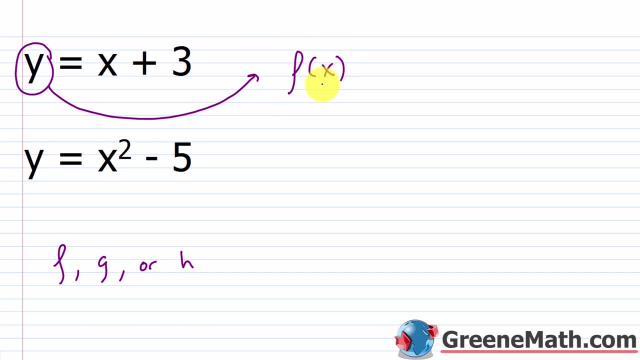 the function depends on f of x, So you're going to have f of x. So you're going to have f of x. So f of x now equals x plus 3.. So there's no difference between this and this, other than I. 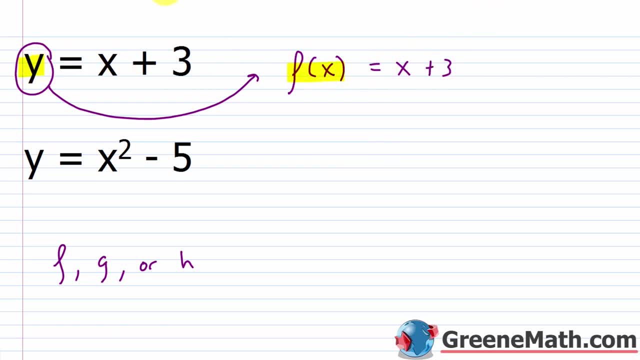 replaced y with f of x, And I could do it over here as well. Instead of y, let me just write g of x. So g of x equals x squared minus 5.. So I replaced y with g of x. So there's really nothing. 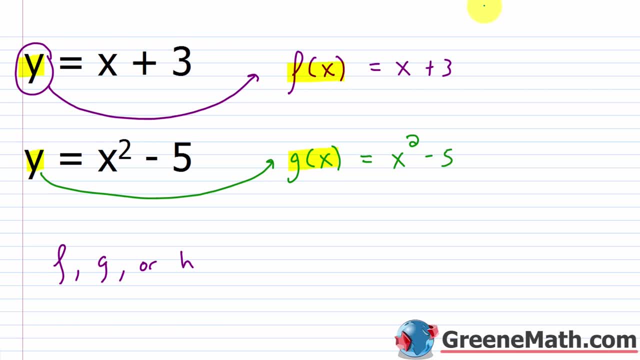 to be confused about here. It's something that's very, very easy. You just have to get used to it. I'm just replacing y with f of x, Or I'm replacing y with g of x, Or I could have replaced y with, let's say, h of x. I'm just saying that I have a function that's dependent. 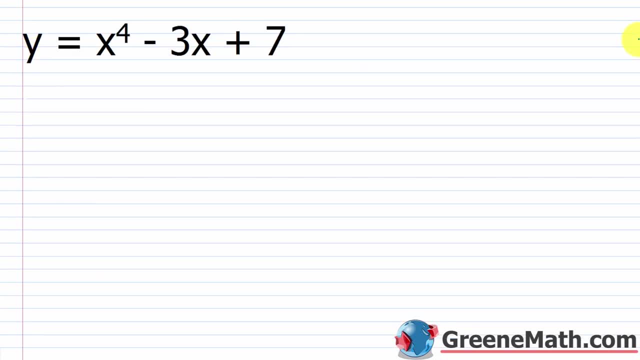 on the value that you give me for x. So as another example, let's say I saw y equals x to the fourth power minus 3x plus 7.. I could write this using function notation, As: f of x is equal to everything is the same, just x to the fourth power minus 3x plus 7.. 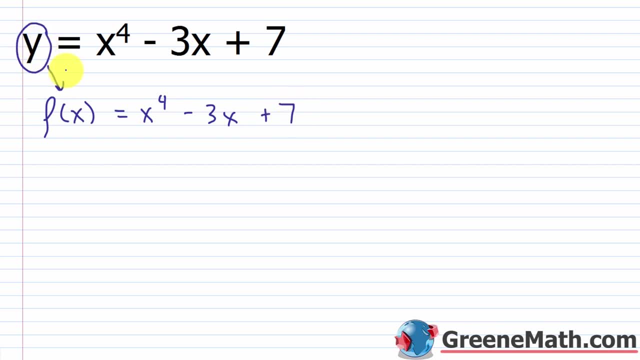 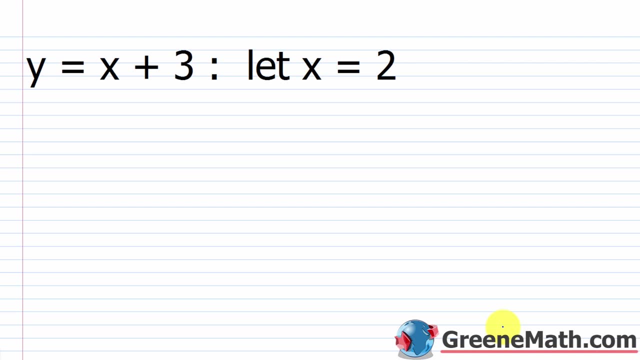 Super, super simple. I just replaced y with f of x. All right, so this notation can immediately be used to evaluate a function for a given x value. So in the past we've done this. okay, It's the same thing. We're not learning anything new, It's just a different way to notate it. 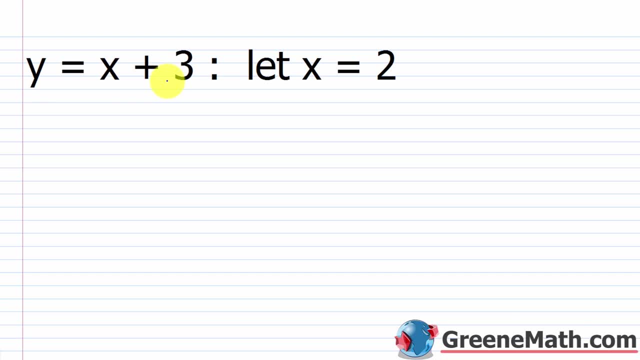 So let's say you saw, y equals x plus 3.. And I said, let's be equal to 2.. What would y be? Well, you would just say, okay, y equals. I would plug in a 2 for x and I would say: y equals 2 plus 3, which is 5.. So then we know. 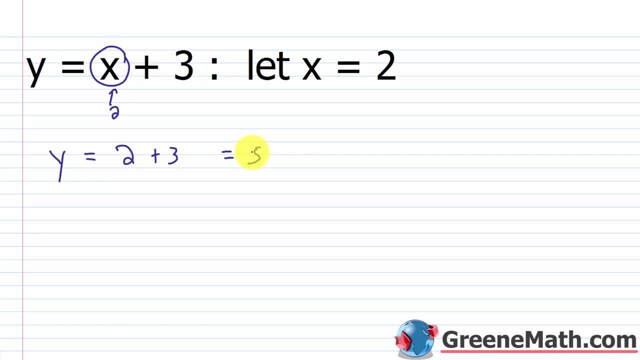 that if x is 2, y is 5.. We've been doing that forever. Now, when I change this up again, students go crazy and go. what do I do? The notation now will be: f of x is equal to x plus 3.. 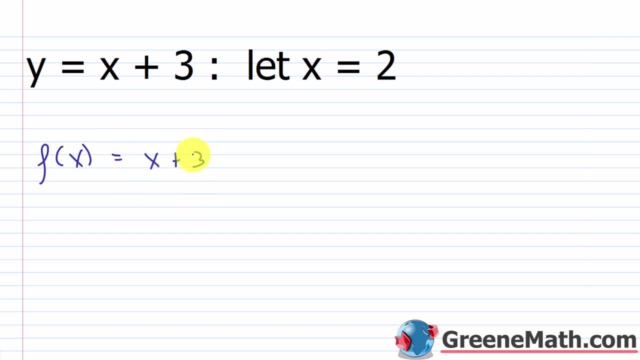 Again, I haven't done anything special. All I've done is I've taken y and I've replaced it with f of x. okay, Nothing special is going on. Now the notation to say: let x be equal to 2, we would say f of 2,. okay, So you have your f. 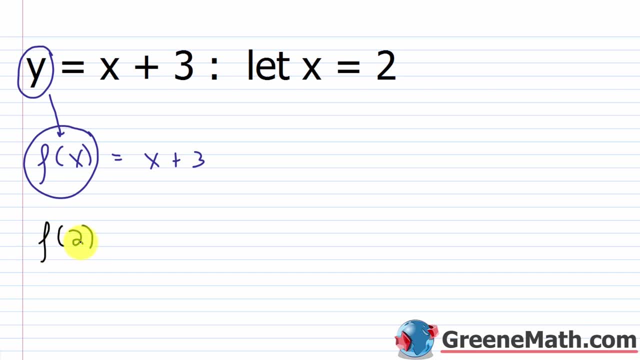 inside the parentheses You have the value that you want x to take on. So f of 2 is equal. to replace x with a 2, then plus 3.. So f of 2 is 5.. This is just saying what is the function's value. 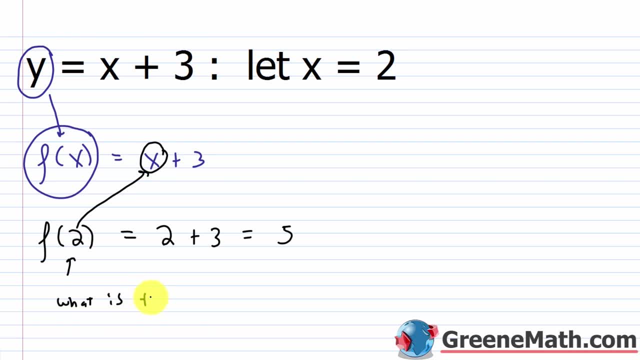 when x is 2?? What is the value when x is 2?? We can see the function has a value of 5 when x is 2.. So let's say I tried another value. Let me erase all this. Let's say that I wanted to let x be. 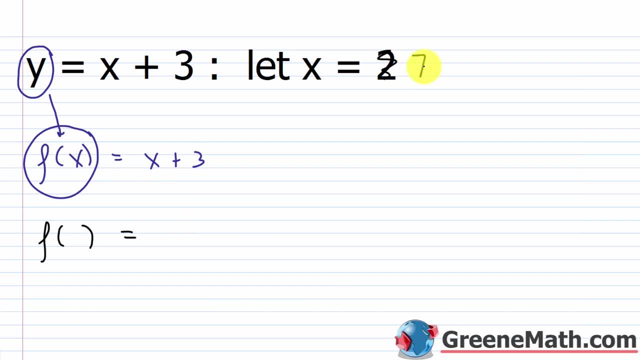 equal to, I don't know, 7.. So how would I ask for that? Well, I would say I want f of 7.. Whatever value you put inside the parentheses, you're just saying, hey, if x was 7,. 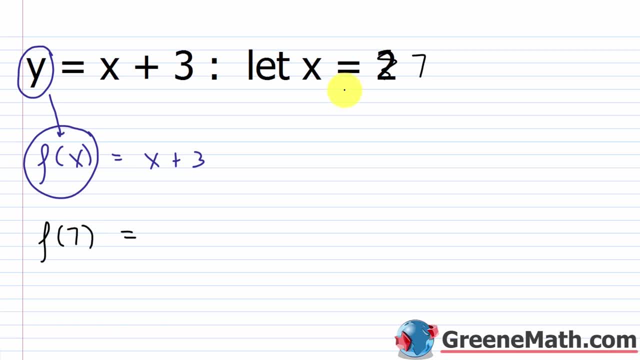 what is the function's value? It's the same thing as saying: let x be equal to 7 and find out what y is equal to Same thing, okay. So the function's value when x is 7, we replace x with a 7,. 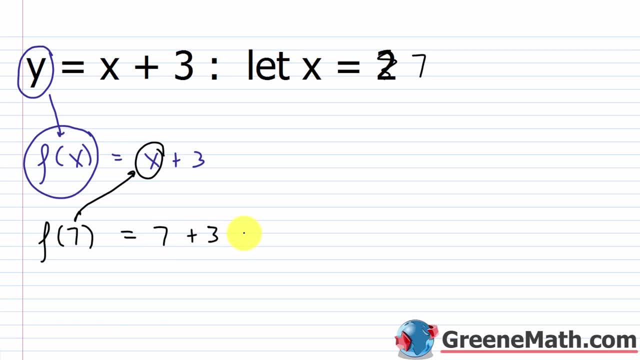 okay, We just replace x with a 7. You'd have 7 plus 3. That equals 10.. So f of 7 is 10.. And again, you can relate that to your earlier procedure. If I just plugged in a 7 for x, 7 plus 3 is 10,. 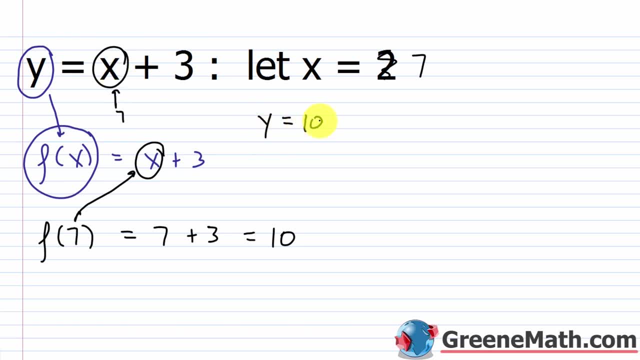 y equals 10.. So y would equal 10.. Or f of 7 equals 10.. The function's value when x is equal to 7 is 10.. That's all we're saying. All right, let's look at a few examples here. This is very, very easy And you won't get into. 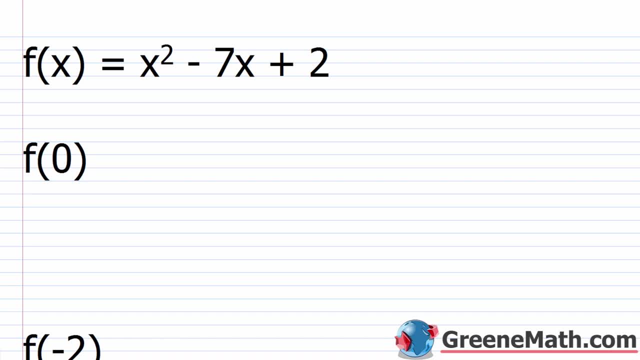 anything harder. When you get to college algebra you're going to talk about the composition of functions. We're not going to get into that here. I'm going to wait until you get to college algebra to deal with that. But I can tell you that it's not much more difficult. But you need to know. 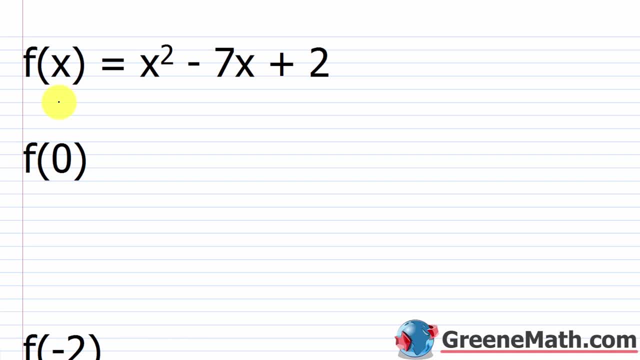 how to do the basics first before you get into the more complicated scenario. So we have: f of x is equal to x squared minus 7x plus 2.. So if I want f of 0, what am I asking for? I'm asking for the function's value when x is 0. So I would simply plug in a 0 here and here. 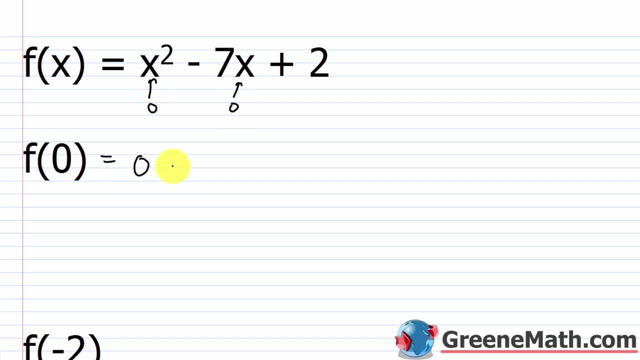 and find out what I get. So 0 squared is 0 minus 7 times 0 is 0 plus 2.. I basically just have 2.. So f of 0, or the function's value when x is 0, is 2.. 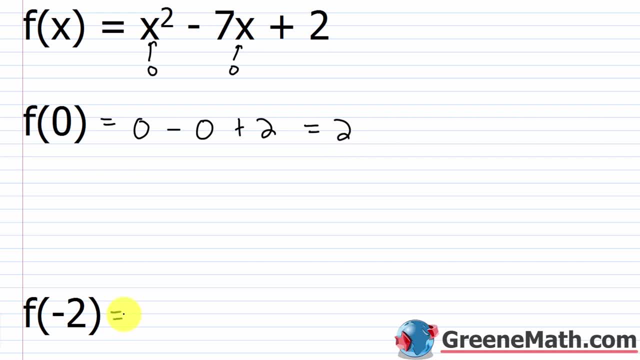 And the next one is: I want to find f of negative 2.. So if I plugged in a negative 2 or x there and there I would have negative 2. And it's inside of parentheses because whatever x is, it's squared. 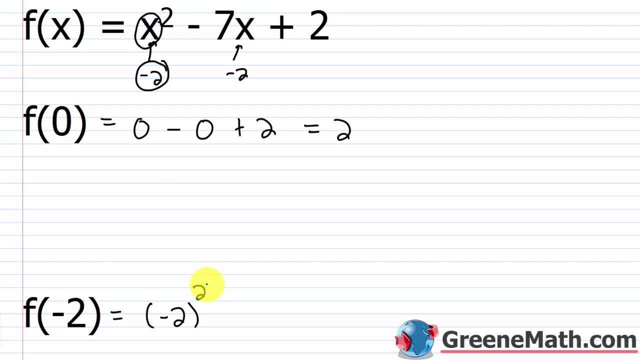 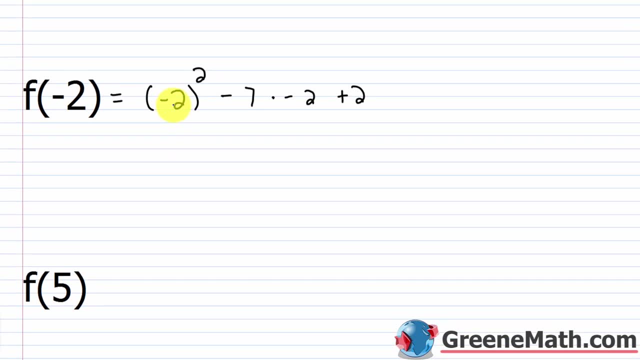 x is negative 2. So we square the negative and the 2.. Then minus 7 times negative, 2 plus 2.. Scroll down a little bit. We'll have negative, 2 squared is 4. Then we have negative 7 times. 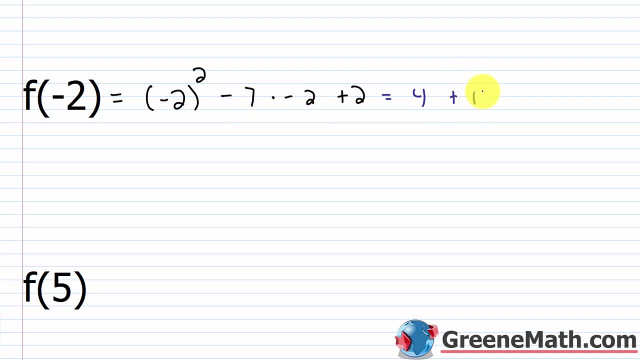 negative 2. That's positive 4. Then we have negative, 2 squared is 4.. Then we have negative 7 times 14.. So plus 14.. Then plus 2.. So 4 plus 14 is 18.. 18 plus 2 is 20.. So we can say the function's value. 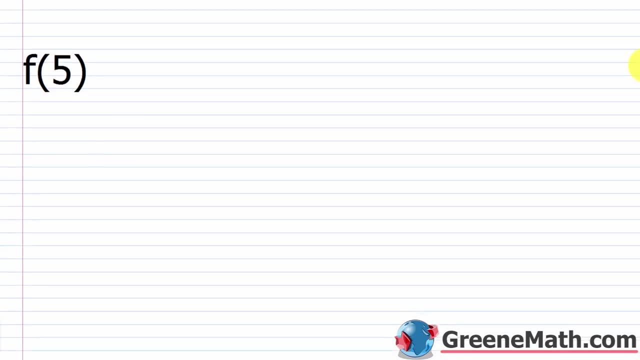 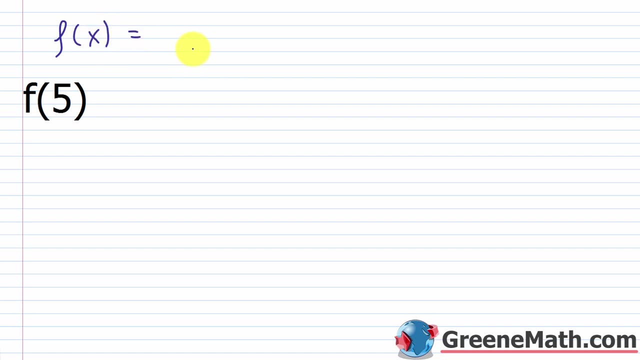 when x is equal to negative, 2 is 20.. All right, So next we want f of 5. And I realize you can't see the function anymore, So let me just rewrite it. f of x is equal to: we have x squared minus. 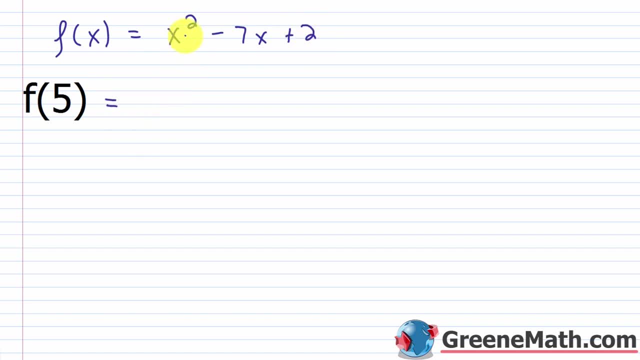 7x plus 2.. So f of 5 would be what? Plug in a 5 here and here You'd have 5, squared minus 7 times 5 plus 2.. 5 squared is 25.. So you'd have 25 minus 7 times 5 is 35 plus 2.. 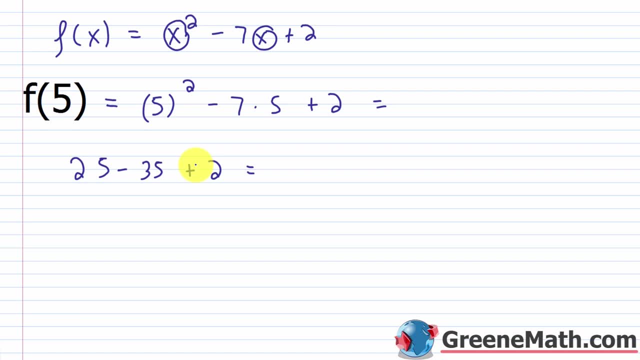 So 25 minus 35 is negative 10.. Negative 10 plus 2 is negative 8.. So f of 5 is negative 8. Again, the function's value when x equals 5.. All right, So now we want f of 9. And again, I'm just going. 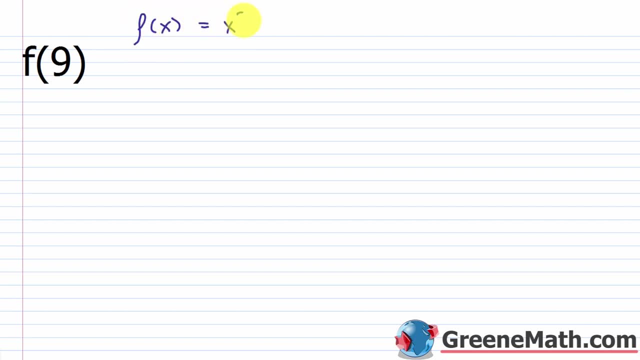 to write my function, f of x is equal to x squared minus 7x plus 2.. So f of 9 is what I'm just going to replace x with a 9 here and here. So I would have- let me kind of write this down here- 9. 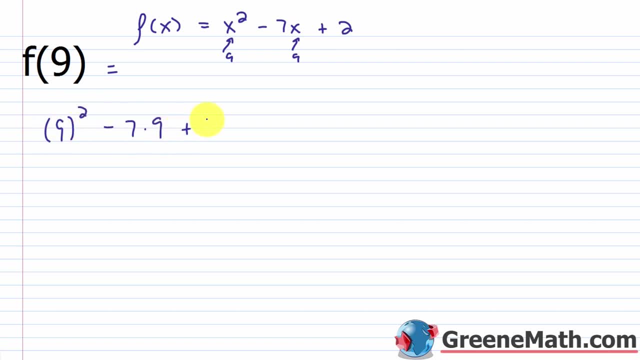 squared minus 7 times 9 plus 2.. 9 squared is 81 minus 7 times 9 is 63 plus 2.. So the easy way to do this is to add 8 to 9.. So I'm going to write: f of x is equal to x squared minus 7 times 9 plus 2.. 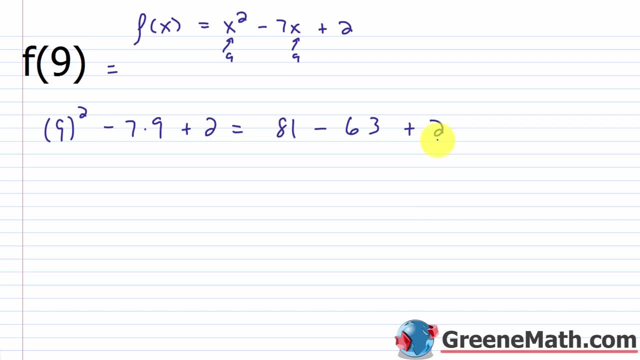 81 and 2. first, 81 plus 2 is 83. Then 83 minus 63 would be 20.. So f of 9,, or the function's value when x equals 9,, is 20.. All right, let's take a look at another example. So we have f of x is. 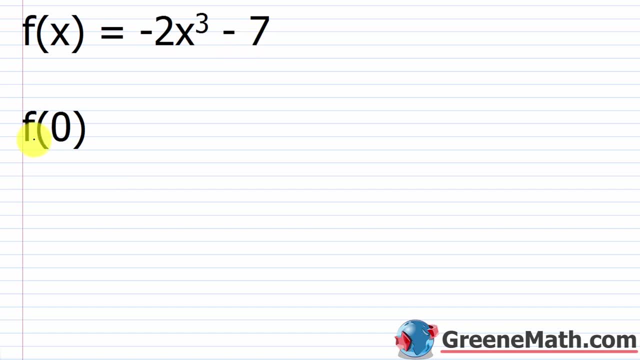 equal to negative 2x cubed minus 7.. We want to find f of 0. So again, all I'm doing is I'm replacing x with that 0. Whatever's inside of parentheses. replace your independent variable with that. So I would have negative 2 times 0 cubed minus 7.. 0 cubed is 0.. Negative 2 times 0. 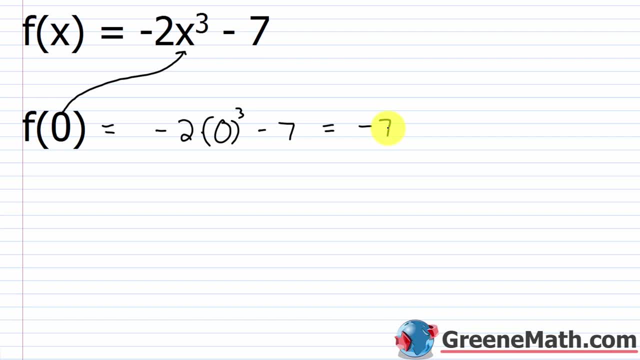 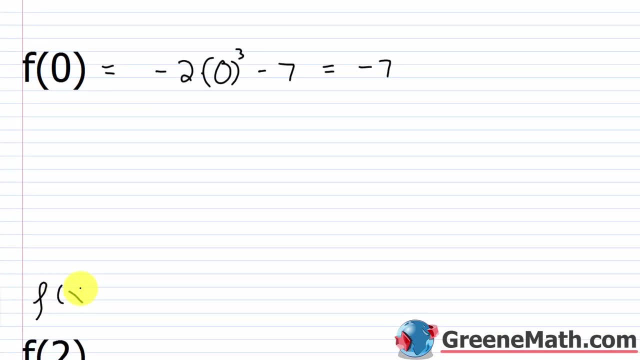 is 0. So you basically have 0 minus 7, which is negative 7.. So f of 0 is negative 7.. So let me rewrite this down here and we'll scroll down. So f of x is equal to negative 2x cubed minus 7.. 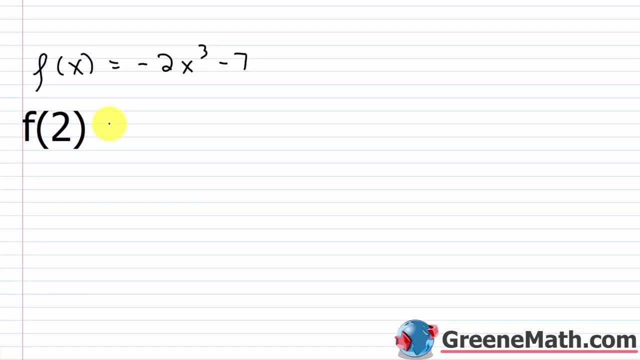 Let's go ahead and scroll down now And I want f of 2.. So f of 2 is what Plug in a 2. So negative 2 times you have 2, that's cubed minus 7.. 2 cubed is 8.. So I'd have negative 2 times 8. 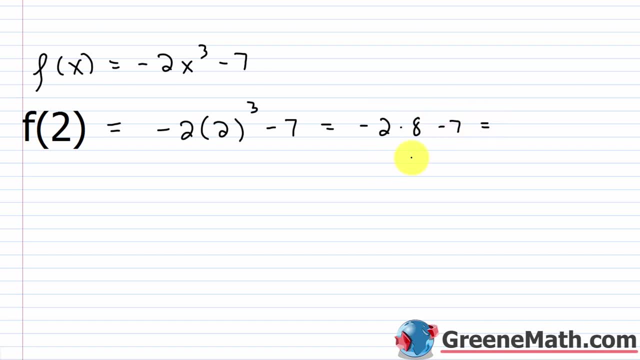 minus 7.. Negative 2 times 8 is negative 16.. So you'd have negative 16 minus 7.. Negative 16 minus 7 is going to give me negative 23.. So f of 2, or the function's value when x equals 2,. 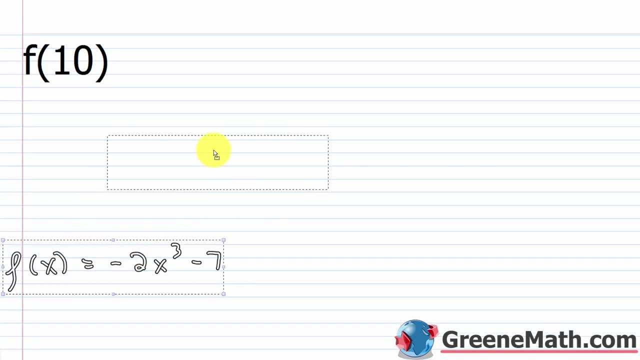 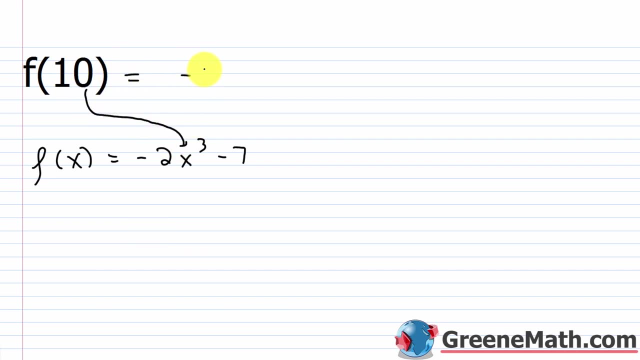 is negative 23.. All right, so let me paste our function here. So f of 10.. So what am I going to do Again? all I want to do is plug a 10 in for x, So I'd have negative 2 times, we'd have 10,. 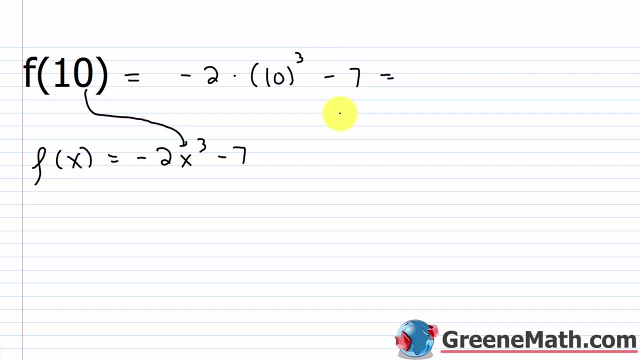 and that would be cubed, then minus 7.. So I'd end up with negative 2 times 10. cubed is 1,000, right, It's a 1, followed by three 0s, then minus 7.. So I know that I would do negative 2 times. 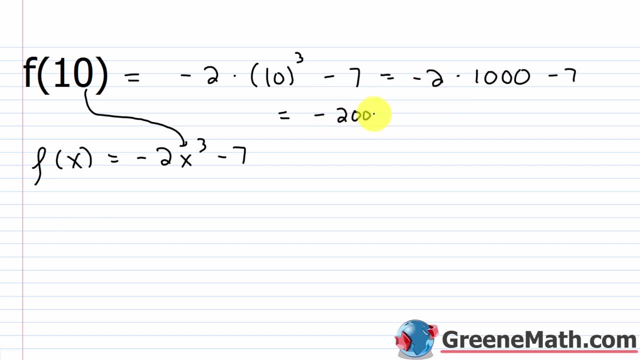 1,000. first, That would be negative 2,000, then minus 7.. This is going to end up being negative 2,007.. So f of 10,, or the function's value when x equals 10, is negative 2,007. All. 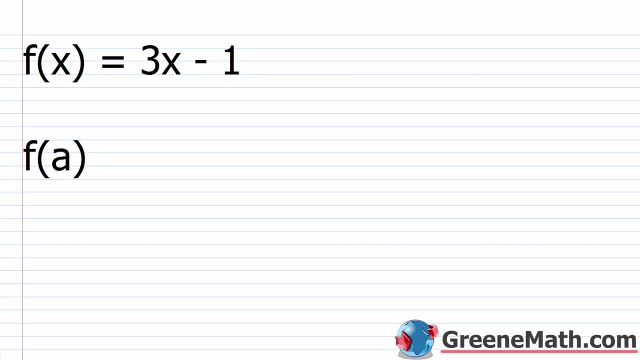 right, let me throw a little bit of a curveball at you. This is something that really trips students up. So I've explained kind of the basics, and when you use numbers it's easy to kind of start getting a hold of that. You can wrap your head around it: everything is fine And everything. 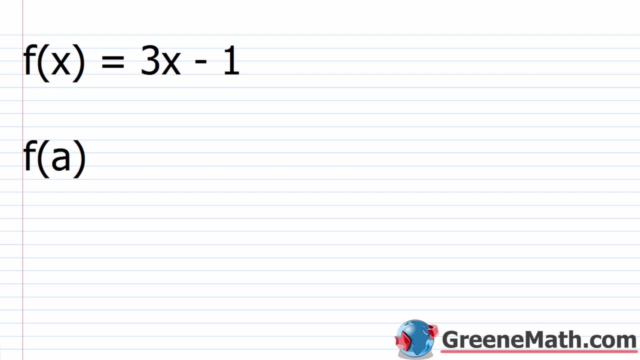 is fine, up until you see another variable that's inside the parentheses, So I'm going to show you this. So let's say you have f of x is equal to 3x minus 1, and you see f of a- I can't say how many. 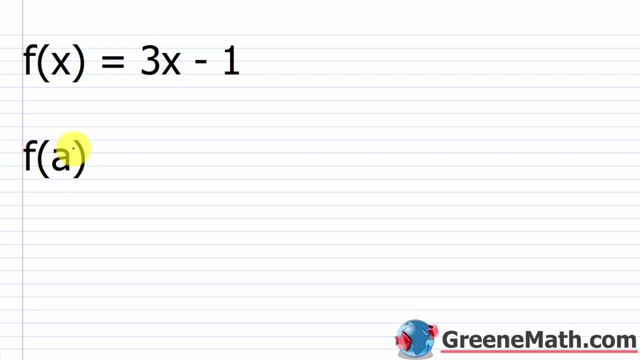 students go ballistic and go. what do I do? It's the same thing. This is what I want to plug in for this. So just like, if you had a 3 there, if I had f of 3, I would plug a 3 in for x. 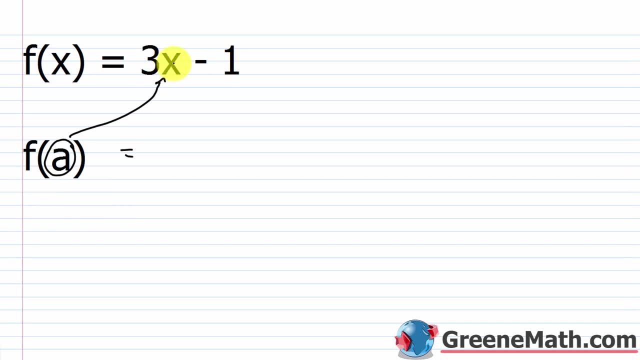 right. And then I would just evaluate: Well, if I have f of a plug an a in for x, I'd have 3 times a minus 1.. So again, if I had f of x, I'd plug a 3 in for x. So if I had f of a plug an a in for x, 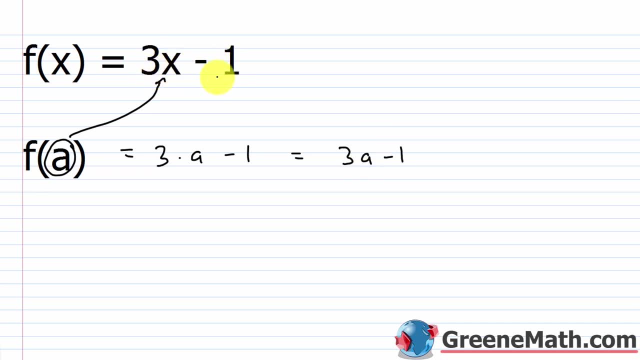 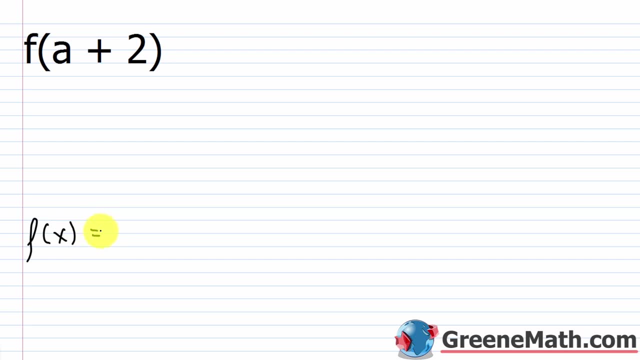 I'd have 3 times a minus 1.. And then I would just go back and look at the function's value. If x was equal to a, it would be 3a minus 1.. That's easy to see. You have one x there, just replace it with. 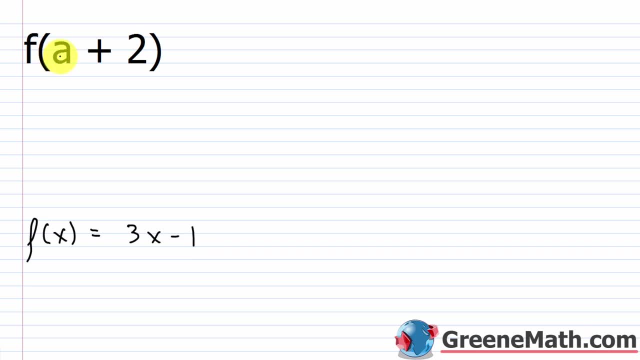 an a instead of 3x minus 1, you've got 3a minus 1.. So it's very, very easy to do that. So again, our function is: f of x is equal to 3x minus 1.. 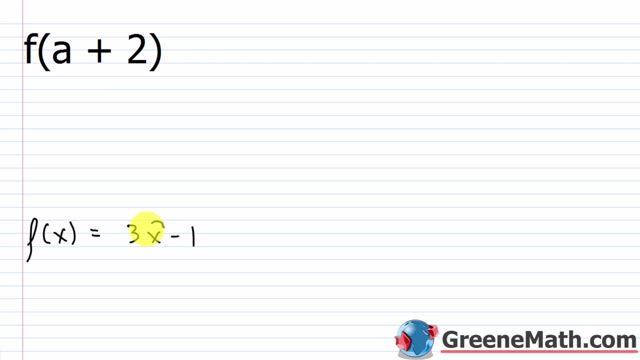 If I have f of a plus 2, I plug in an a plus 2 for x, So a plus 2.. Use parentheses because it's going to stop you from making mistakes. Just use parentheses whenever you substitute things in, okay, It'll stop you from making silly errors. So I would have 3 times the quantity a plus 2,. 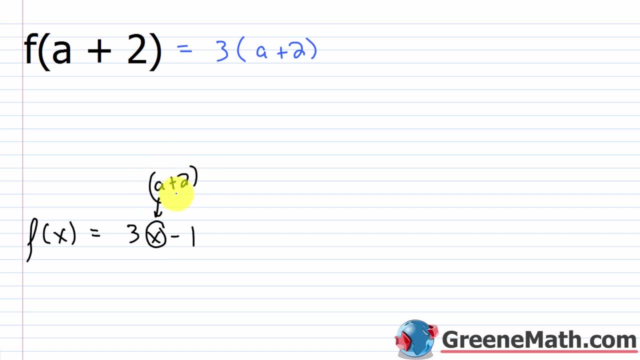 because, remember, 3 is multiplied by x. x now represents this quantity. So unless I use my distributive property, I'm not going to get the right answer right, And I don't want to see this because you'll get the wrong answer. Students will go okay. 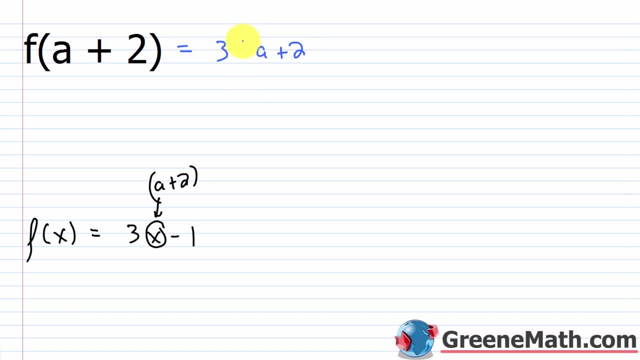 it's 3a plus 2.. No, it's 3 times the quantity a plus 2.. That's 3a plus 6, okay, So that's what you want. So then I have minus 1 there. All I did was I substituted in for the x. there, I plugged. 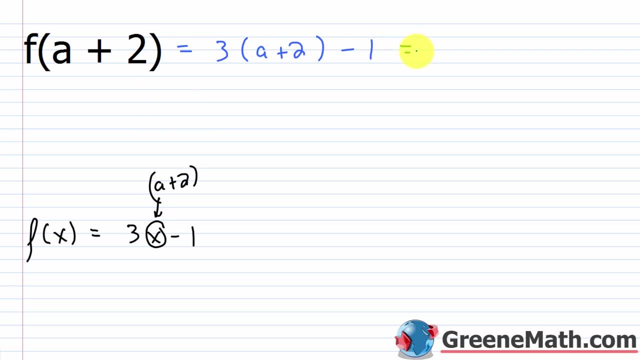 in an a plus 2.. All I did, All right. so now use my distributive property: 3 times a is 3a, then 3 times 2 again is 6, then minus 1.. So then 3a plus 2.. 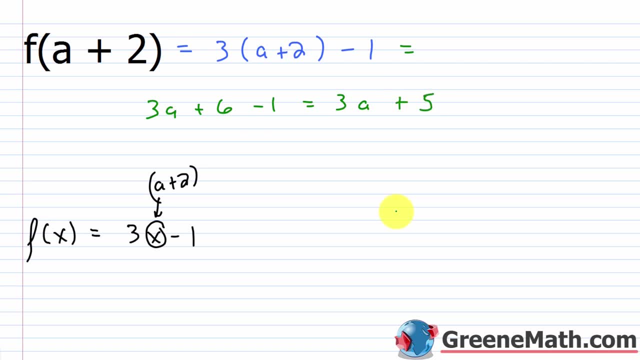 a plus 6 minus 1 is just 5.. So the function's value when x is equal to a plus 2 is 3a plus 5.. Again, all I did was I replaced x with a plus 2.. That's it. No magic, no trickery. 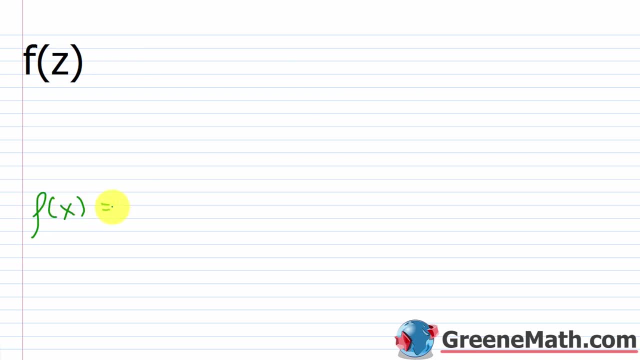 nothing like that. All right, so one more time We have: f of x is equal to 3x minus 1.. What if I saw f of z? What do I do? Again, take this and plug it in here. All I'm doing, So I would have 3, plug in a z for x minus 1.. All I did was I replaced the x. 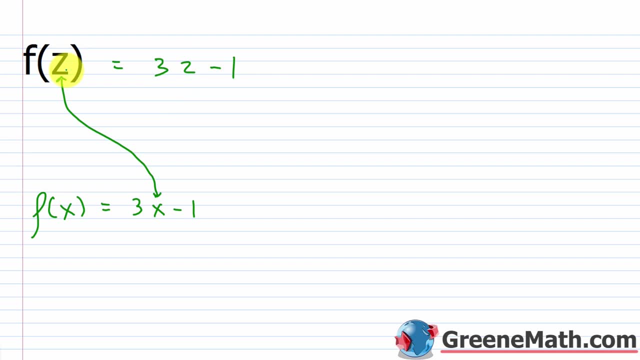 with a z, because this is what it told me to do. So the value of this function, when x is z, is 3z minus 1.. That's it. I just swapped the x with a z. All right, let's take a look at another one now. 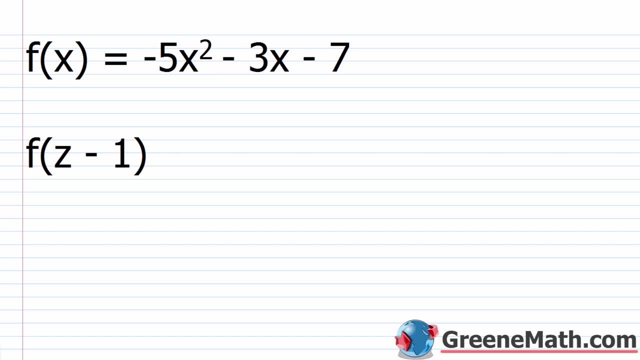 So we have: f of x is equal to negative 5x squared minus 3x minus 7, and I'm given f of z minus 1.. So again, I'm just going to take this and plug it in here and here and see what I get. So I would have negative 5 times. I'm going to put this inside. 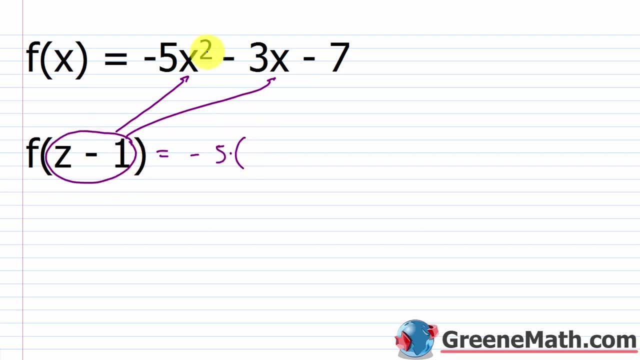 of parentheses, because I want to multiply by this squared, So z minus 1, that quantity has to be squared and then multiplied by negative 5.. Then minus 3 times this quantity: z minus 1.. Again, use parentheses: minus 7.. So we know how to do this quickly. We use our special products formula. 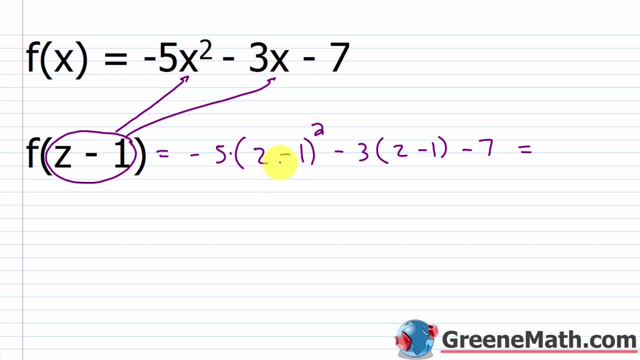 Z minus 1, if we square that quantity we get z squared minus 2z plus 1.. So I'd have negative 5 times that quantity, Again, z squared minus 2z plus 1.. Then you think about this as negative 3 times z, that's minus 3z. 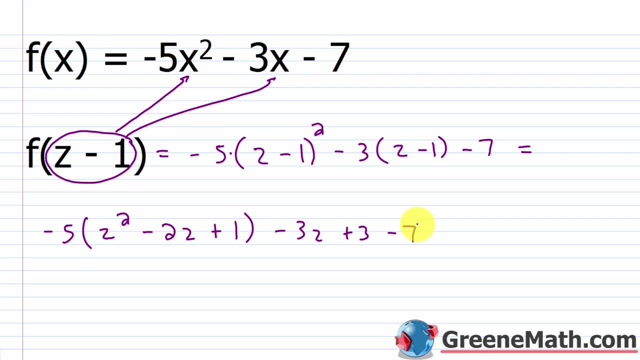 And then negative 3 times negative 1 is plus 3, and then minus 7.. All right, so now I want to use my distributive property here. Negative 5 times z squared is negative 5z squared, Then negative 5. 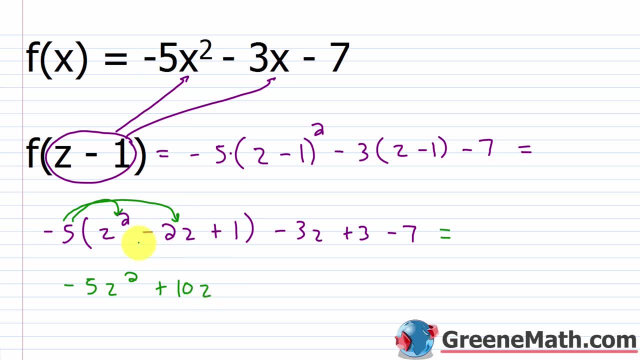 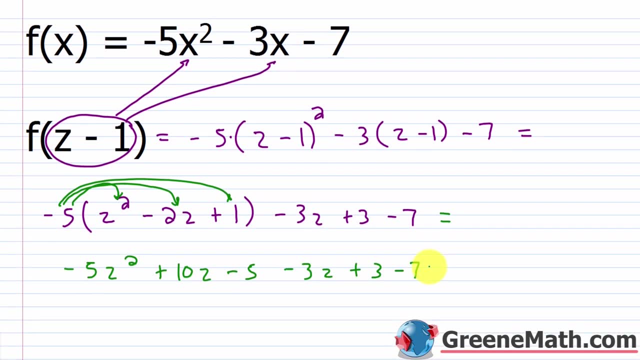 times negative 2z is plus 10z, Then negative 5 times 1 is minus 5.. Then you have minus 3z plus 3 minus 7.. So now we're just combining like terms. So I start out with negative 5z squared. I can't do anything with that. 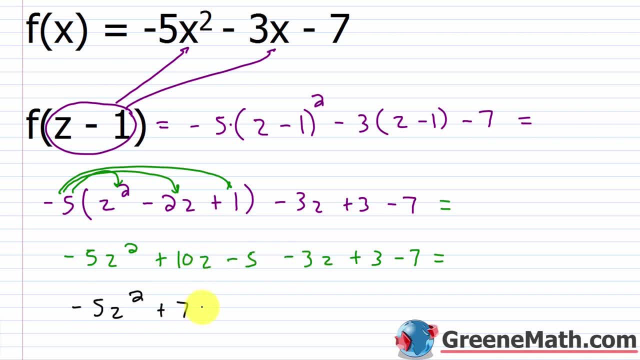 Then I've got 10z minus 3z, that's plus 7z. Then I've got negative 5 plus 3, that's going to give me negative 2.. And then negative 2 minus 7 is minus 9.. So the function's value when x is z. 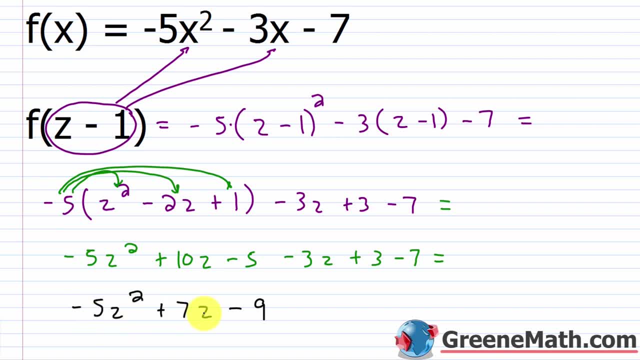 minus 1, that's minus 9.. So the function's value when x is z minus 1, that's minus 9.. That's minus 9.. I get negative 5z squared plus 7z minus 9.. All right, so lastly, let's talk about another source. 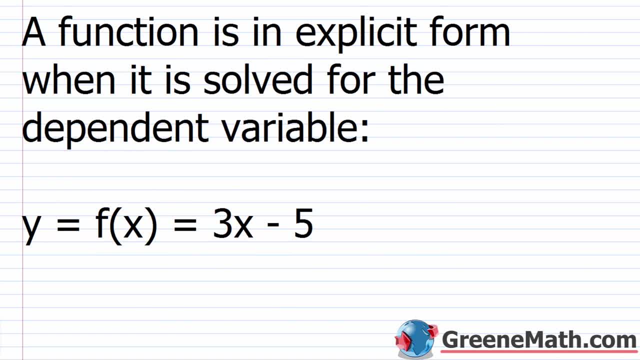 of confusion. So a function is generally represented in what's known as explicit form. So this is when it's solved for the dependent variable. So y equals f of x, which equals 3x minus 5.. I just took y and replaced it with f of x. It's all I've done. But y is on one side of the equation. The expression 3x minus 5 is on the. 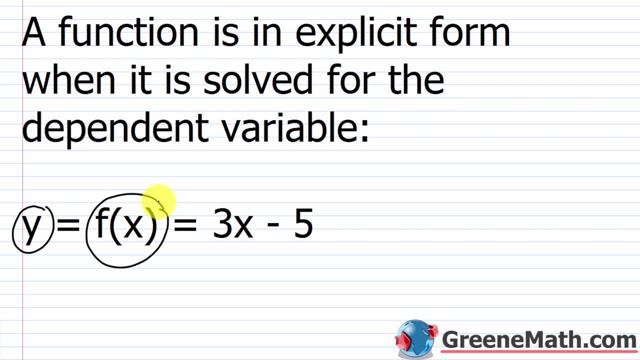 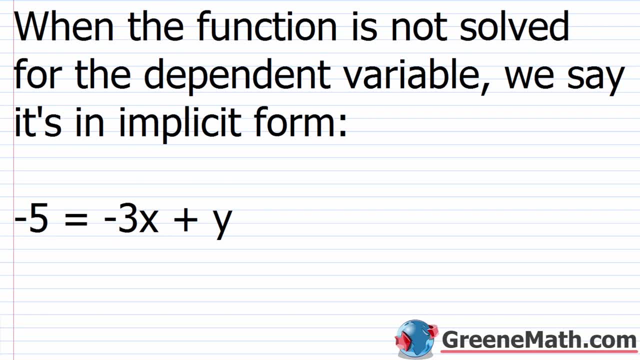 other Solve for y. So when we have this, it's easy to just evaluate for a given value of x. Now, in other scenarios, the function is not solved for the dependent variable. So we say that it's an implicit form. okay, Implicit form, So this means the function is not solved for the dependent? 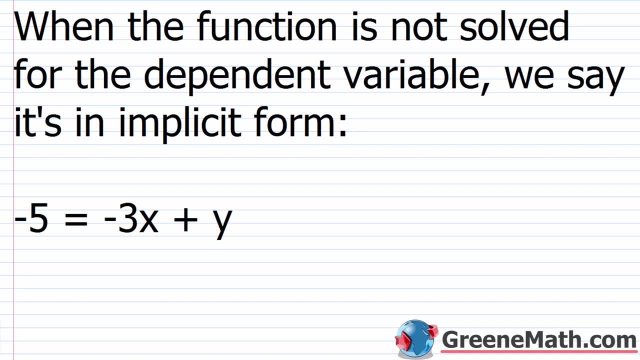 variable. Remember that, As you're going to get to calculus, you're going to hear about implicit differentiation And you're going to be like: what does that mean? What do I do? It means the function is not solved for y And you. 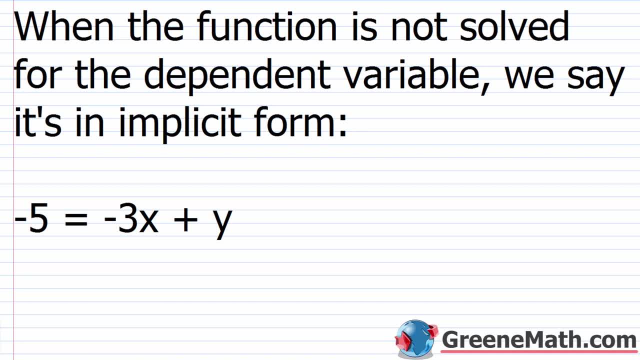 need to find the derivative, but you don't want to go through the process of solving it for y first. So remember that, because when you get to calculus you're going to thank me. All right, So we have an example here. Negative. 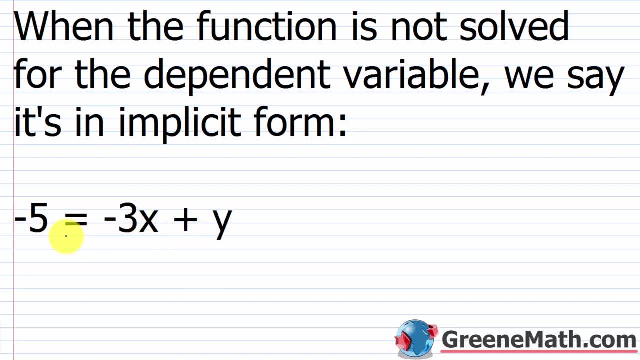 5 equals negative 3x plus y. So what would I do if I wanted to put this in explicit form? Well, I would just solve it for y. Just simply add 3x to both sides of the equation and you're done. It's an explicit form. You would have. 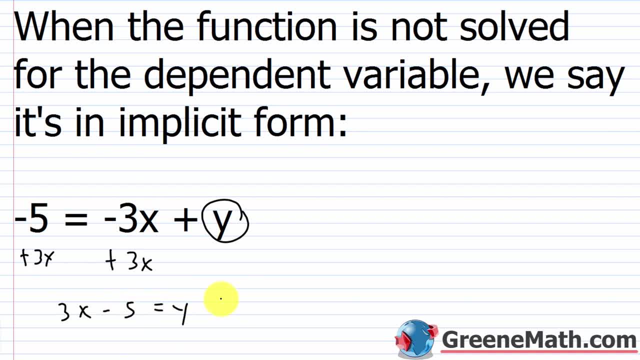 3x minus 5 equals y. Or I could just do this: Simply say y is equal to 3x minus 5.. Using function notation, I could say f of x is equal to 3x minus 5.. Again, all I'm doing is replacing y with f of x, But hopefully you can see the difference. In one case, in explicit form, which we have here, it's solved for the dependent variable y. When it's in implicit form, it's not So. y is just kind of jambled up. It's not on one side of the equation by itself. That's implicit form. 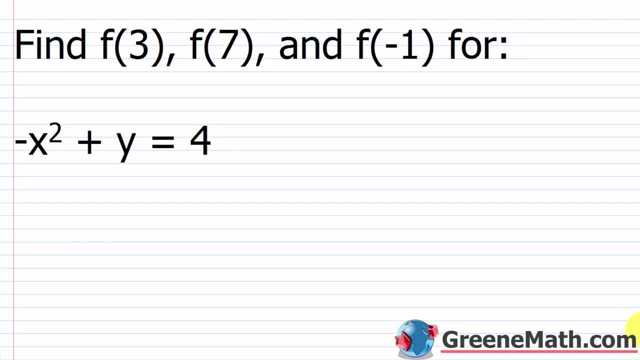 So if you get a problem like this one, you've got to do additional work. So you might be asked to, let's say, find f of 3,, f of 7, and f of negative 1,, 4, and. 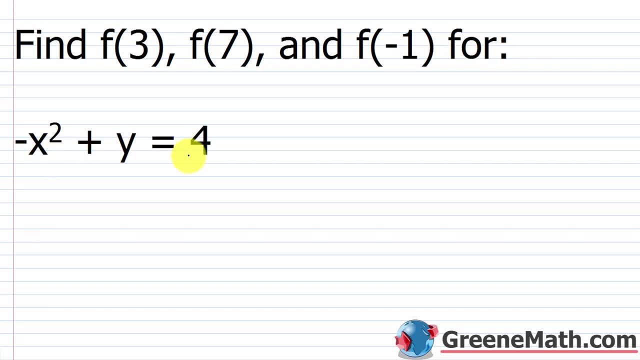 we have an implicit function here. We have negative x squared plus y equals 4.. So what do I got to do? I got to solve it for y first, then replace y with f of x, then do my normal procedure, Okay. 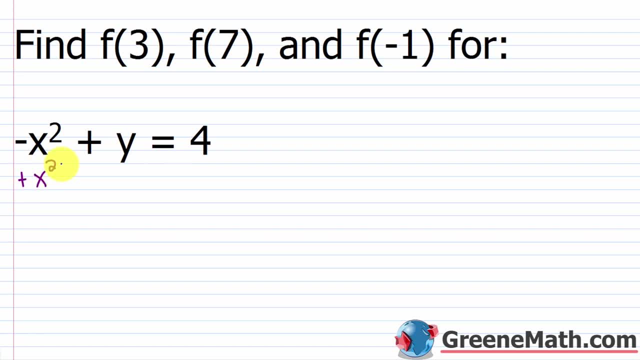 It's not much more work. So I would add x squared to each side of this equation and I would find that y is equal to x squared plus 4.. I can then replace y and say y is a function of x. So I use this notation here and it equals x squared plus 4.. 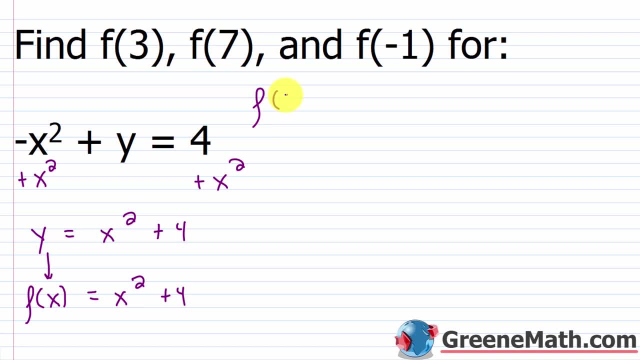 So if I want to find f of 3, what do I do? I just plug a 3 in here. So f of 3 is what It's: 3 squared, which is 9, plus 4, which is going to give me 4.. 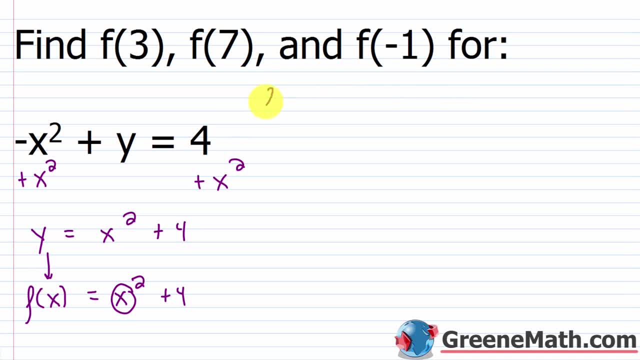 So f of 3 is 13.. If I want f of 7, plug a 7 in for x, So I'd have 7 squared plus 4.. 7 squared is 49.. 49 plus 4 is 53.. 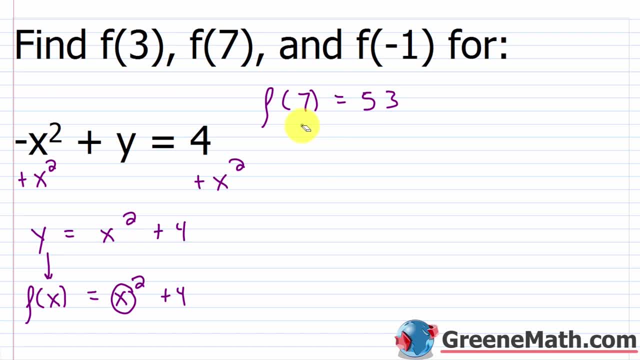 So f of 7 would be 53. Then, lastly, if I wanted f of negative 1, well, I'd plug a negative 1 in for x. Remember I'm squaring whatever x is, So negative 1 has to be inside a parentheses. 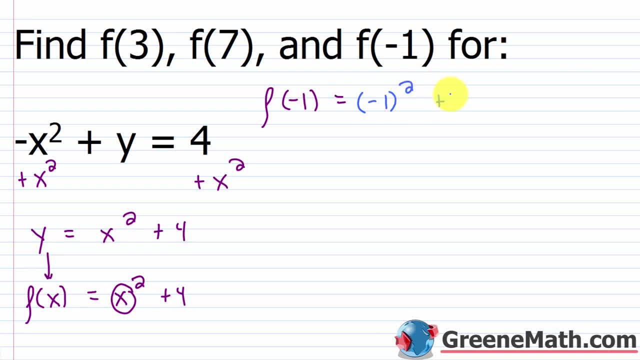 Because I'm squaring the negative and the 1.. So negative: 1 squared plus 4.. Negative: 1 squared is 1.. 1 plus 4 is 5.. So f of negative, 1 is 5.. All right, let's take a look at one more of these. 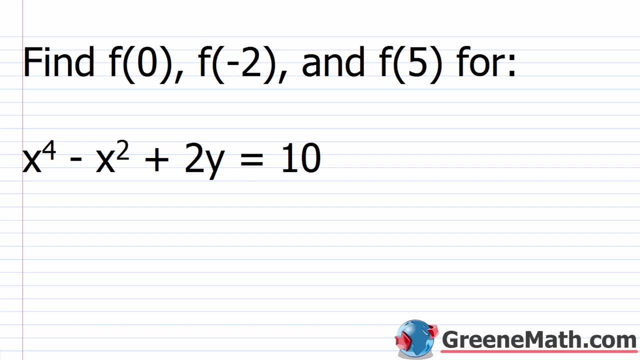 And I made it a little bit harder to solve for y. So we want to find f of 0,, f of negative 2, and f of 5, 4.. And we have x to the fourth power minus x, squared plus 2y equals 10.. 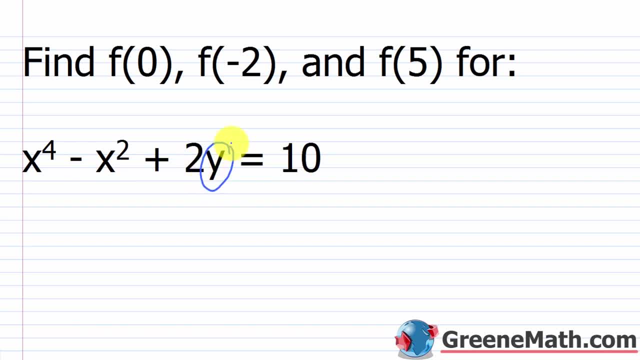 Again, solve for y. Replace y with f of x. Very, very simple. So let me subtract x to the fourth power from both sides of the equation. Let me add x squared to both sides of the equation. We'll just start with that. 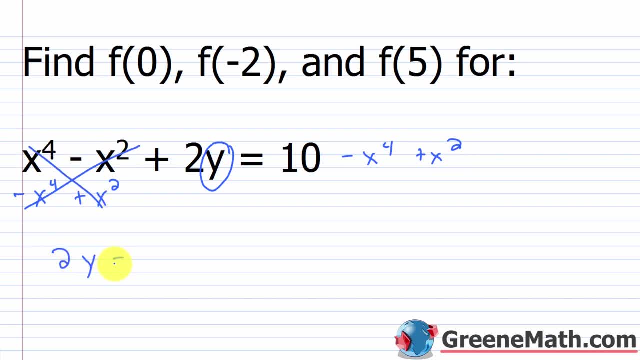 So this is going to cancel. I would have: 2y is equal to: let's write negative x to the fourth, power plus x, squared plus 10.. Now to get y by itself. what do I got to do? I got to divide everything by 2.. 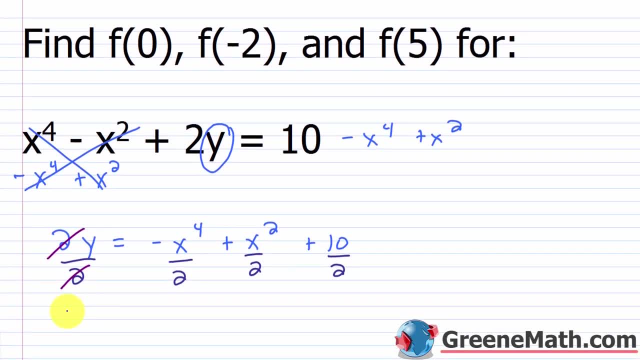 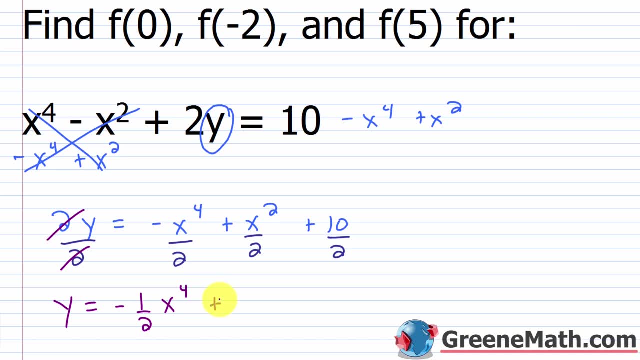 OK, So we divide both sides by 2.. This cancels with this And I have. y is equal to, You'll have a negative And you could write 1 half times x to the fourth power plus you can write 1 half times x. squared plus 10 over 2 is 5.. 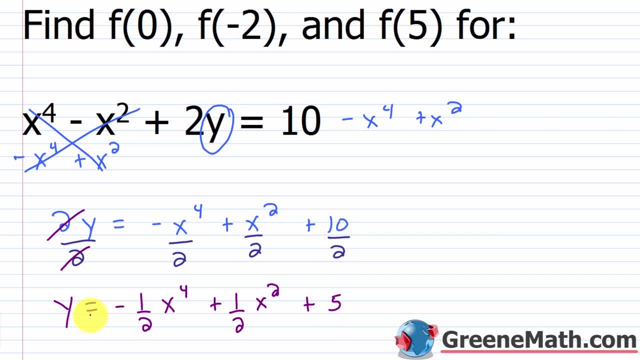 So I can go ahead and replace this y with f of x. I can say: let me just erase all of this, We don't need it anymore. I can say y is f of x. OK, They're the same And this is equal to y. 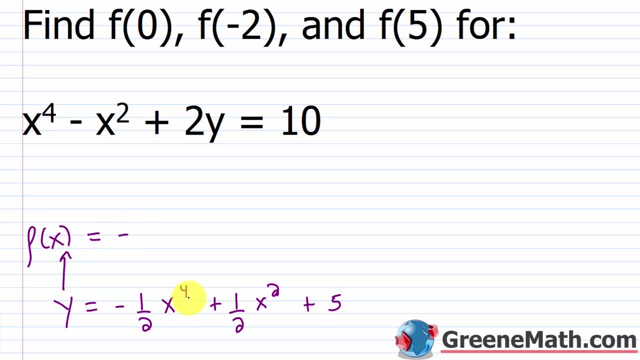 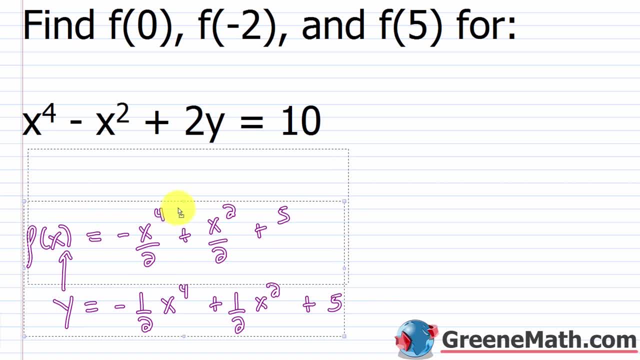 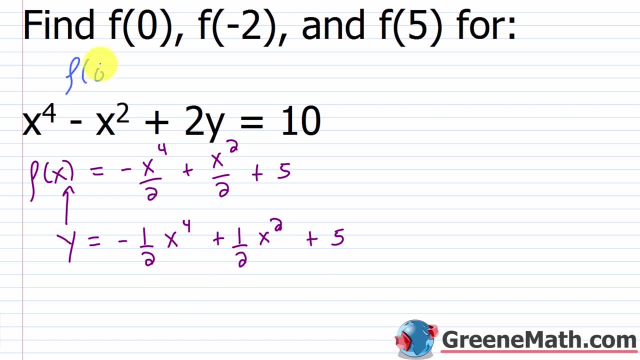 Let me kind of move these up a little bit, OK, So now, if I want to find f of 0,, f of 0, what do I do? Plug in a 0 for each x. So I know that 0 to the fourth power is 0. 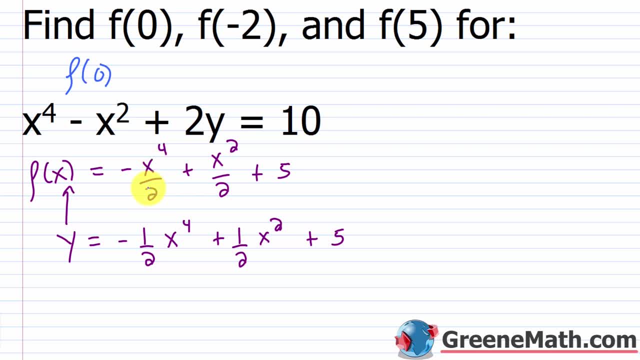 The opposite of that would still be 0.. Divide by 2, I get 0.. 0 squared is 0.. Divide by 2, I get 0.. So these two would cancel themselves. You're just left with 5.. 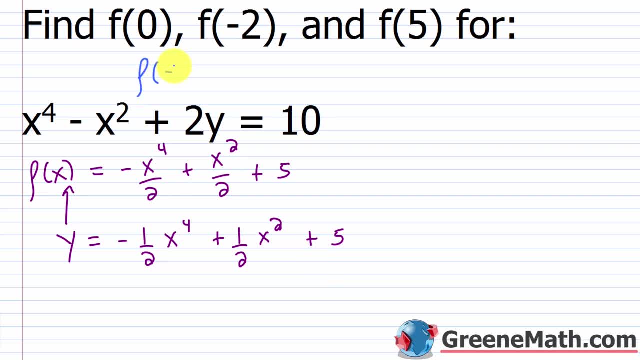 f of 0 is 5.. So now I want to find f of negative 2.. So f of negative 2 is what I would plug in, a negative 2 for each x, So I'd have negative and then in parentheses I'd have negative 2 to the fourth power. 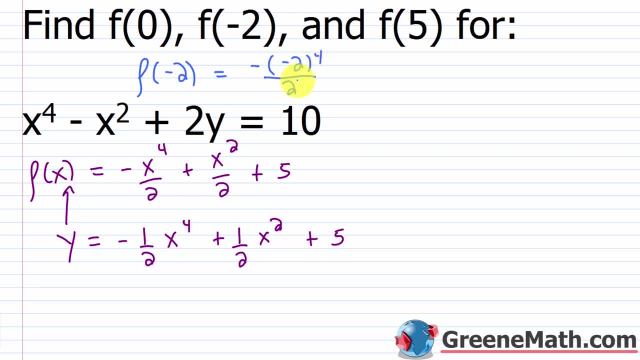 Make sure you use parentheses when you're substituting. It'll stop you from making mistakes. This is over 2.. Then plus, I'm going to have negative 2 inside of parentheses, squared over 2, then plus 5.. 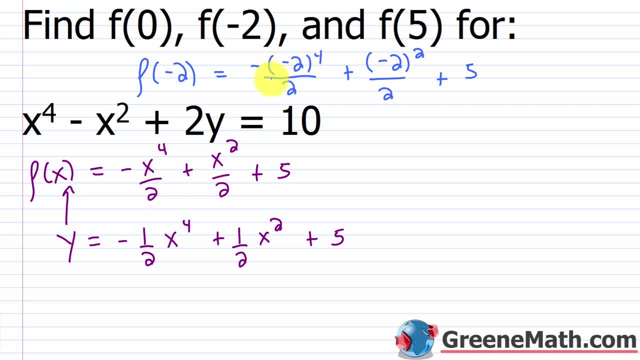 So negative 2 to the fourth power is 16, but the opposite of 16 would be negative 16.. So negative 16 over 2 would be negative 8.. So this would be. I'm going to make a little line there. 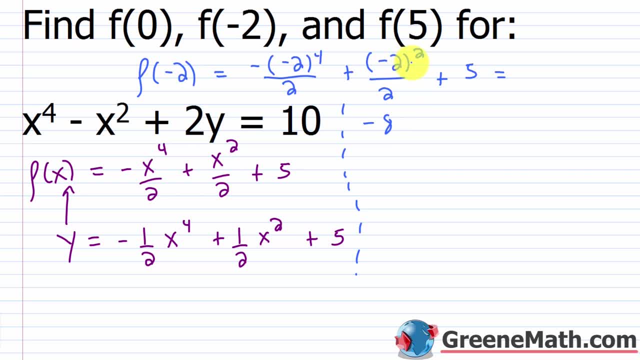 This would be negative 8, and then negative 2. squared is 4.. 4 over 2 is 2, so plus 2, plus 5.. So negative 8 plus 2 would be negative 6.. Negative 6 plus 5 is negative 1.. 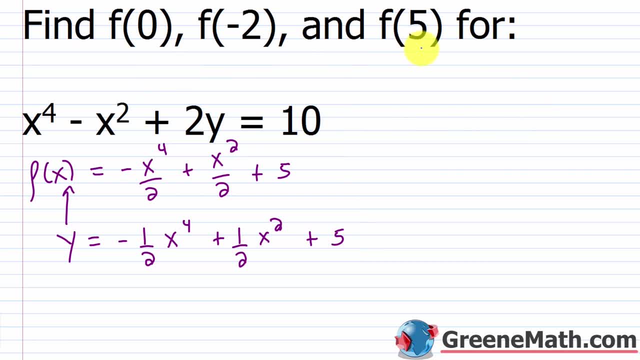 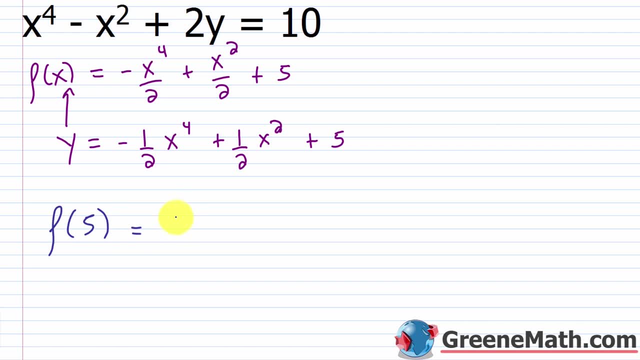 So f of negative, 2 is negative 1.. Then, lastly, we want f of 5.. Let me kind of scroll down a little bit to get that one going. So f of 5.. So I would have negative. in place of x, I'd plug in a 5, and that's to the fourth power over 2,. 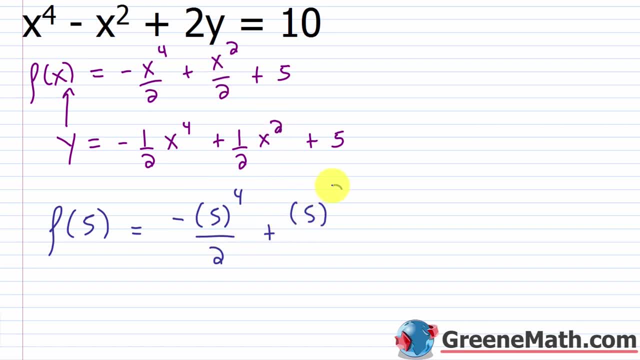 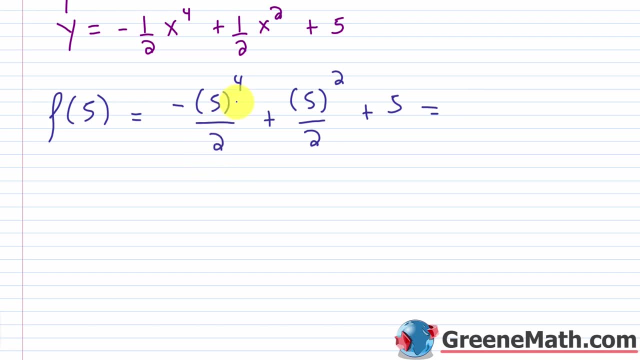 plus I have 5, that's going to be squared and that's over 2, then plus 5.. All right, so let's scroll down and get a little room going. So 5 to the fourth, power is 625.. 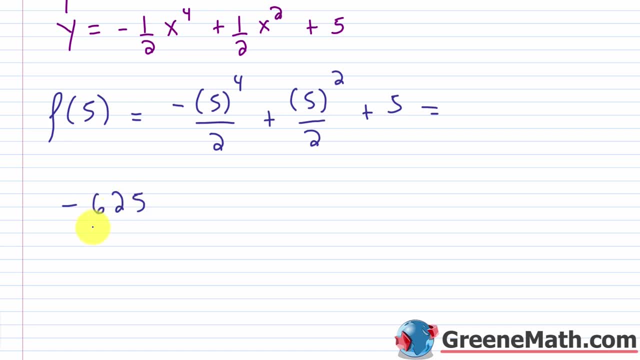 So I'd have negative 625 over 2, and then 5 squared is 25.. So I'd have plus 25 over 2, then plus 5.. We'll have a common denominator here. Negative 625 plus 25 would be negative 600.. 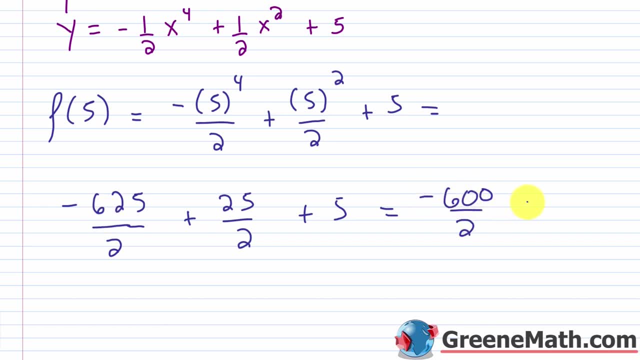 So this would be negative 600 over 2 plus 5.. We know negative 600 over 2 would be. So this would be equal to negative 300, and then plus 5, this would end up giving me negative 295.. 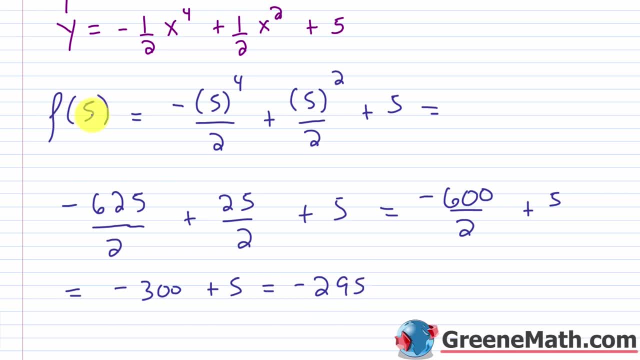 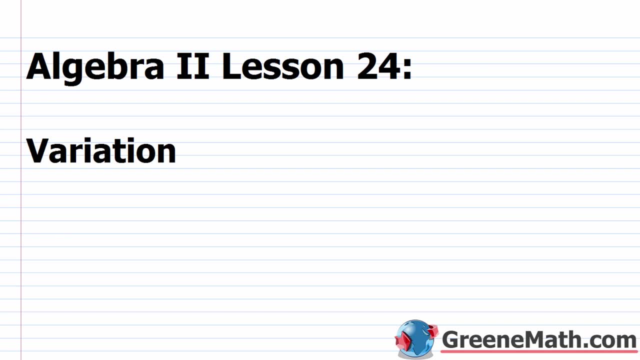 So f of 5, or once again, the function's value when x is 5, is going to be negative: 295.. Hello and welcome to Algebra 2, Lesson 24.. In this video we're going to learn about variation. 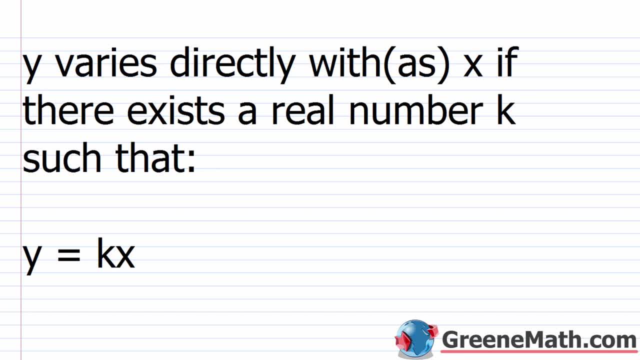 So if you've taken an Algebra 1 course, you've heard about variation in the past. Here we're going to talk about the things we've talked about in the past. We're going to talk about the things we've talked about in the past. 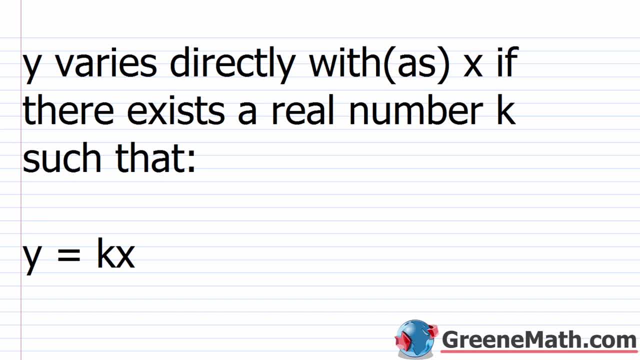 We're going to talk about an Algebra 1, but we're going to learn about something known as joint variation as well, So I want to start out by talking about direct variation. So this is the easiest type of variation to understand. It's the most common type of problem that you're going to get when you talk about variation in an Algebra 1 course. 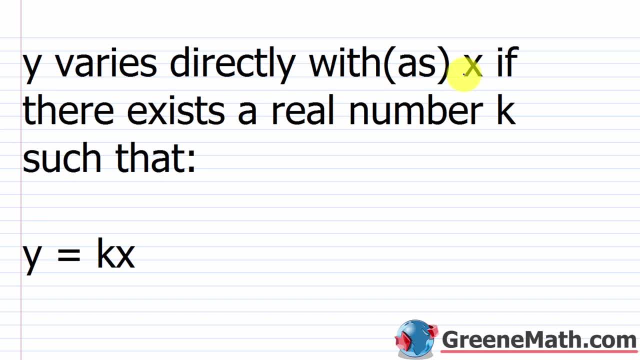 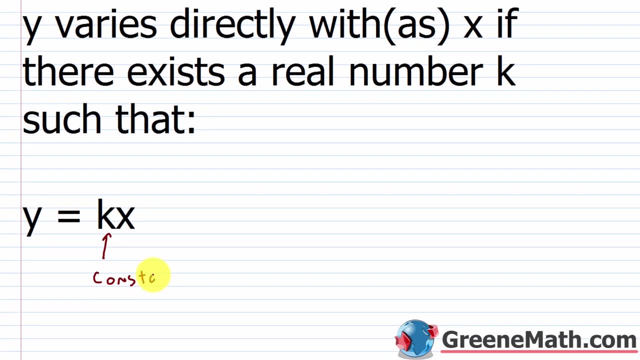 So y varies directly with x, or you might read: y varies directly as x, if there exists a real number, k, such that y equals k times x. So this k here has a special name. It's called the constant of variation, And it doesn't change. 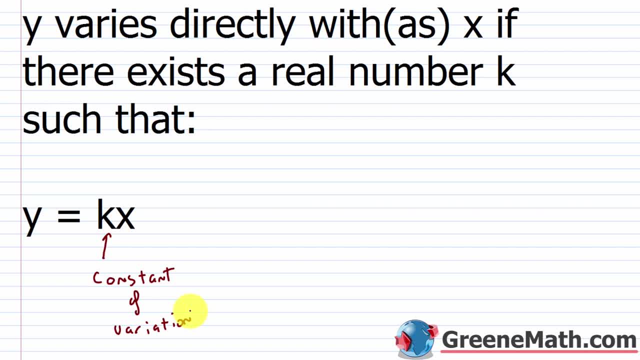 The constant of variation. You might also read this in your textbook. or your teacher might say the constant of proportionality. It's the same thing. So y equals k times x. So let's get a little example going. Let's say I had y equals 2x. 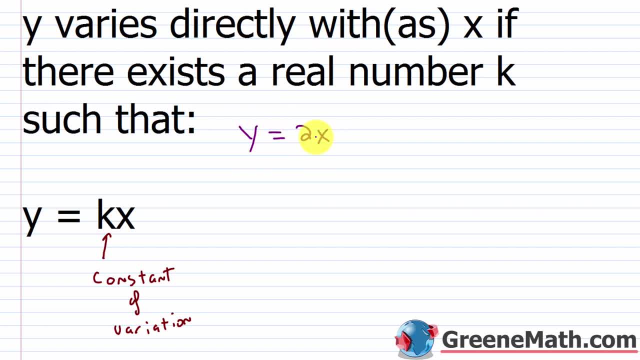 What does this do, if we think about this? Well, if I choose a number for x, I plug it in, I multiply it by 2, and I get a number for y. So if I make a little table of values here, if I chose, let's say, 1 for x, y would be 2.. 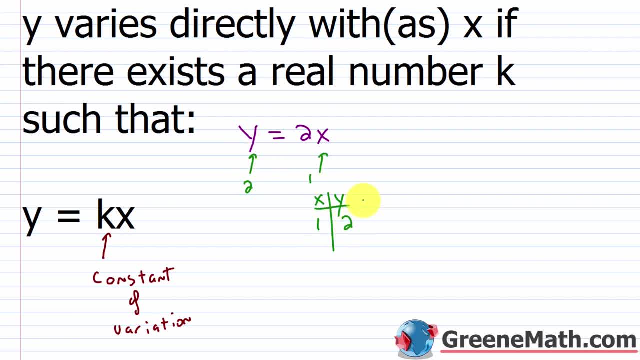 So x equals 1, y equals 2.. If I chose, let's say, 2 for x, y would be 4.. 2 for x, y is 4.. If I chose, let's say, 3 for x, we all know y would be 4.. 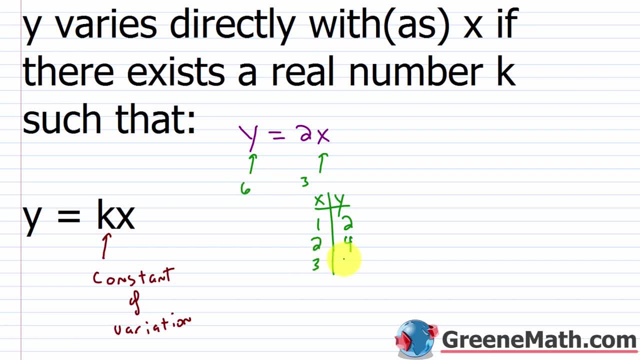 2 for x. y is 4.. y would be 6.. x is 3, y is 6.. Alright, so what can we see from these three ordered pairs here? Well, we see that as x increases by 1 unit, y increases by 2 units. 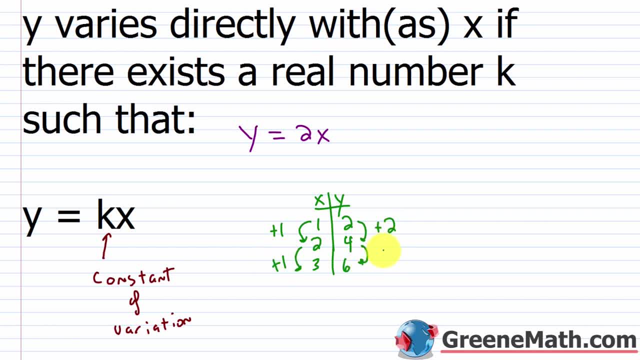 x increases by 1, y increases by again 2.. So what we can say specifically here: if k again- that's this right here, in this case that's 2, is greater than 0,, as x increases, y increases. 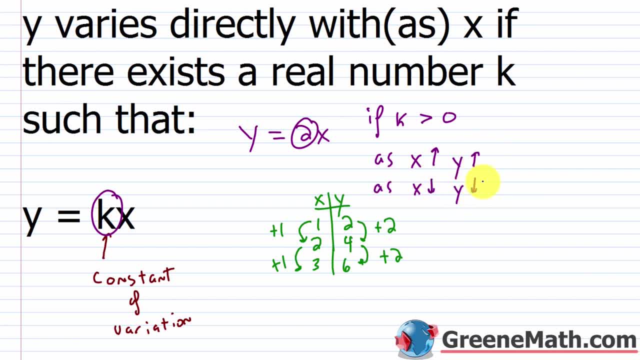 As x decreases, y decreases. This is the case with direct variation. Now to get more specific: as x increases by 1 unit, y increases by k units. We see that here x increases by 1 unit. it goes from 1 to 2.. 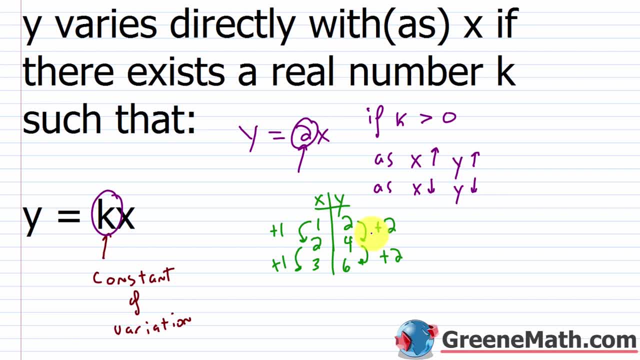 y increases by 2 units. it goes from 2 to 4.. Now we've already seen something like this. Think about the fact that we talk about slope-intercept form all the time. If I look at, y equals mx plus b. 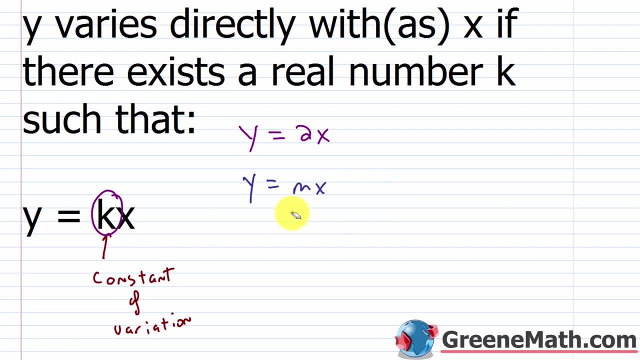 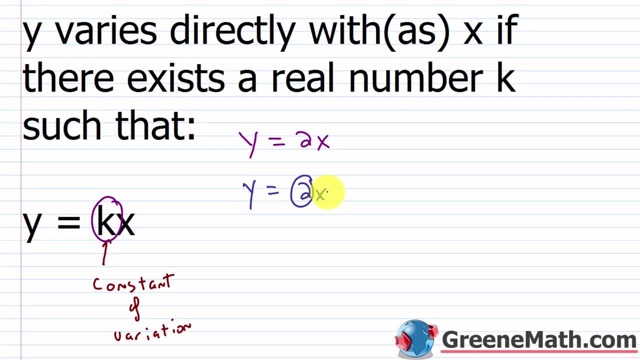 if b was 0 and m was 2, I'd have the same thing there. y equals 2x. So 2 is nothing more than the slope of this line. So if I was to graph, y equals 2x. well, I know the y-intercept is where. 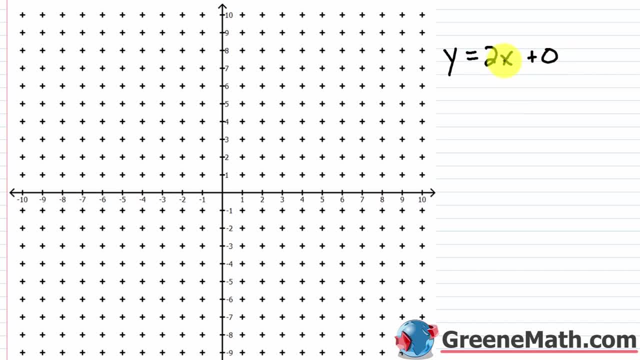 I could put plus 0 here and I'd make it obvious: if I plugged in a 0 for x, I'd get a 0 for y. So the y-intercept is at the origin and my slope is 2.. 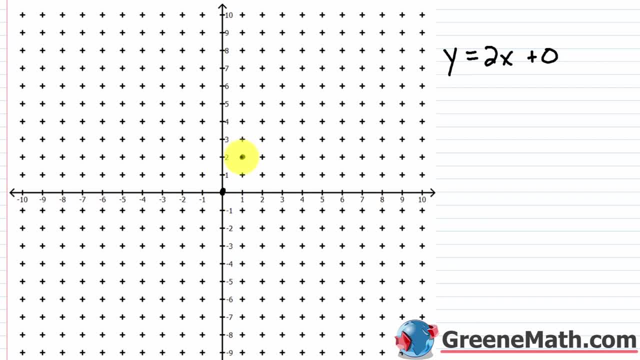 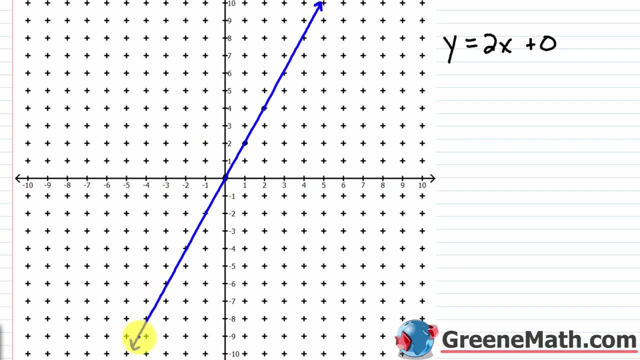 So I would go up 2 to the right 1.. Up 2 to the right 1.. So this would be the graph of: y equals 2x. And again, if I start at a given point, if I go to the right 1,. 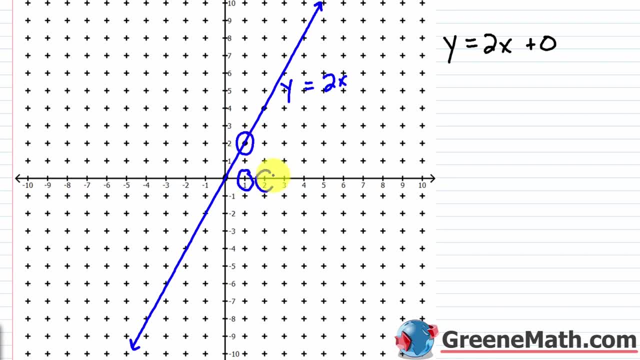 meaning, if I increase my x location from 1 to 2, what happens? Well, to go back to the line I've got to go up 2.. So I went from 1 to 2, my y location goes from 2 to 4.. 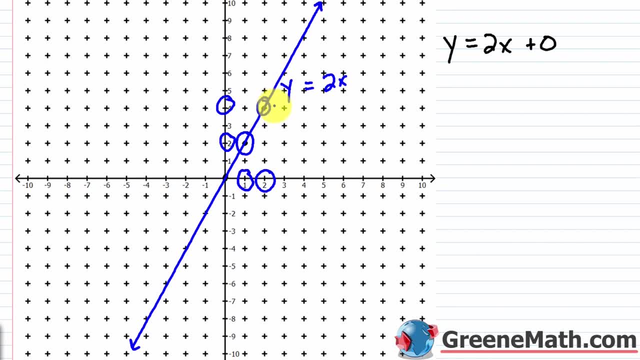 So to the right 1, up 2, back to the line. To the right 1, increase my x by 1, I've got to go up 2 to get back to the line. To the right 1, up 2 to get back to the line. 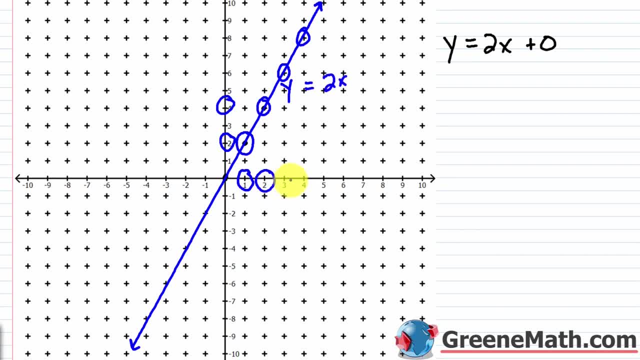 So we can clearly see: as we increase x by 1,, we increase y by 2, or that k, If I had y, equals 7x. as an example: If I increase x by 1,, I'm increasing y by 7.. 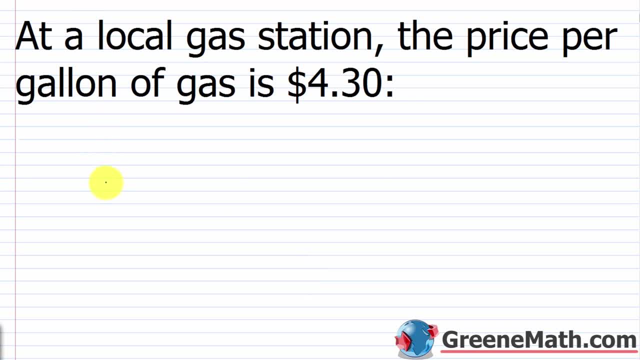 So as a real-world kind of example, suppose you go to a local gas station. So I have at a local gas station the price per gallon of gas is $4.30.. So if I wanted to model how much a person would spend on gas there. 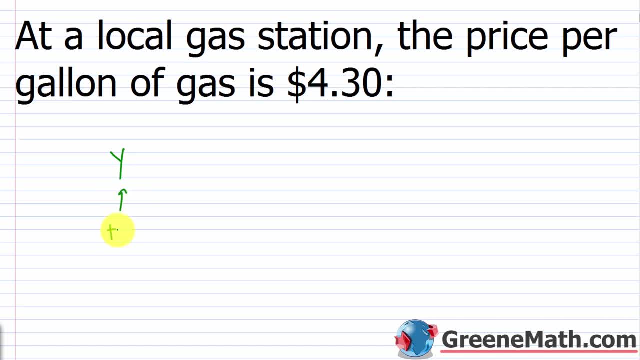 well, I could say y is the total purchase And that's just on gas. that's not if you stop in and get a candy bar And this would be equal to we'd have $4.30 per gallon, so let's put 4.30.. 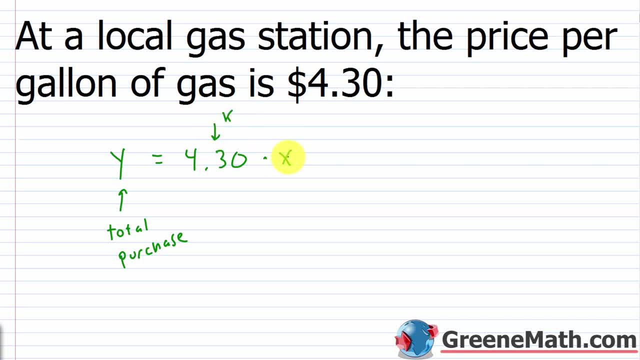 This is representing k and this would be times x, and x would represent the number of gallons. Okay, the number of gallons of gas. So if I buy 1 gallon of gas, I just multiply it by $4.30,. 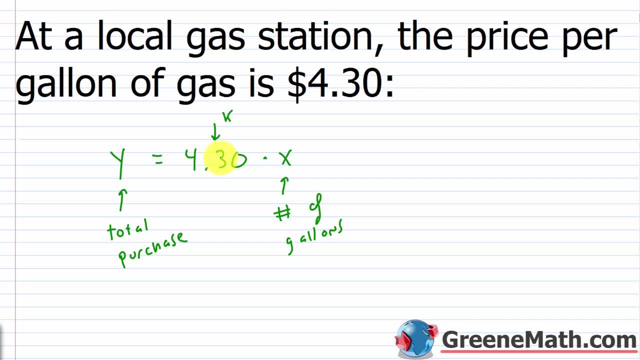 and I know I spent $4.30.. If I buy 2 gallons of gas, I would spend $8.60, because 2 times 4.30 is $8.60.. If I did 3,, I would spend $12.90. 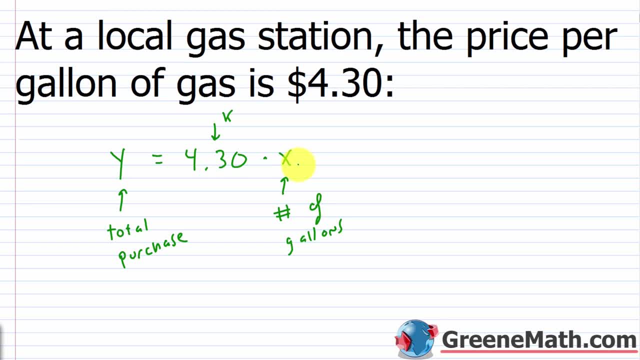 You know, so on and so forth. So as x increases by 1 unit, as x increases by 1, y increases by 4.30.. 4.30.. So again, this is what we're talking about when we talk about direct variation. 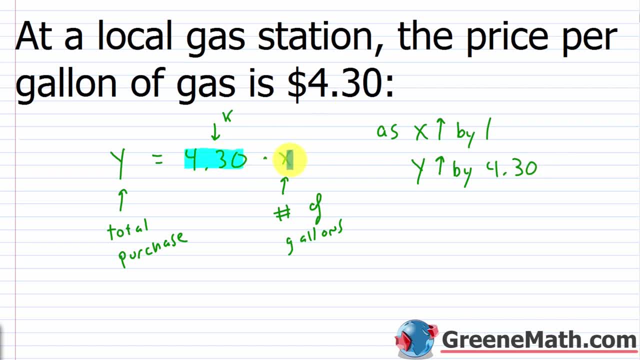 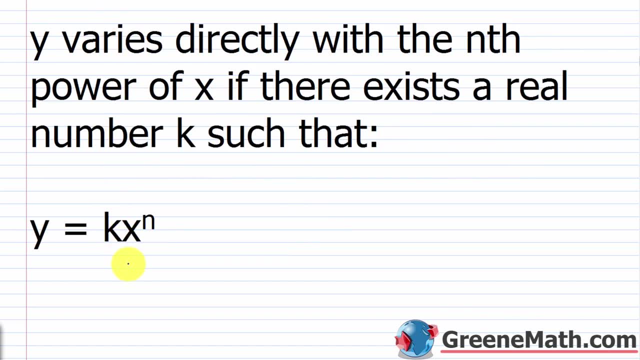 There's a constant value here, that is multiplying x. It will not change. All right, so there's another type of direct variation we're going to see. So y varies directly with the nth power, the nth power of x, if there exists a real number, k. 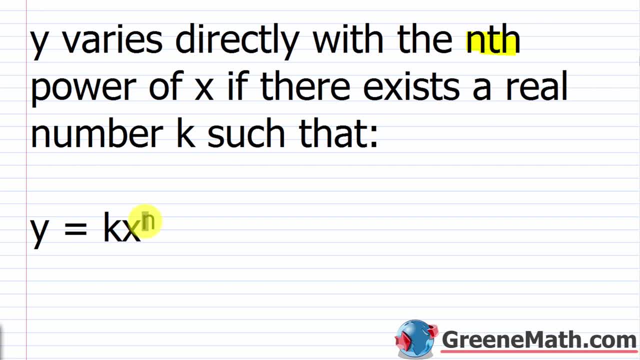 such that y equals k times x to the nth power. So the only thing different here is we're raising x, our independent variable, to a power. So this is known as direct variation as a power. All right, so the next one we're going to run across. 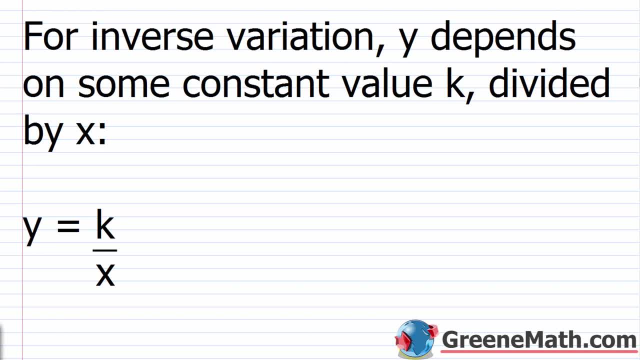 is inverse variation. So for inverse variation now, y is going to depend on some constant value, k divided by x, So I have y equals k over x. So again, this is the constant of variation, And so that doesn't change. Now, as an example of this, 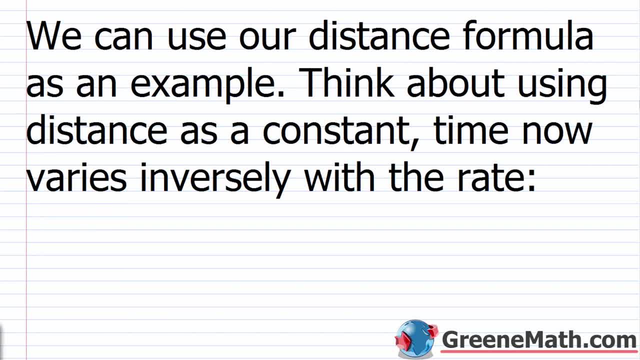 we can think about our distance formula. Okay Now, the distance formula is something we use for the motion word problems that we solve. Distance equals rate of speed times, the amount of time traveled. So d equals r times t, What I have here. 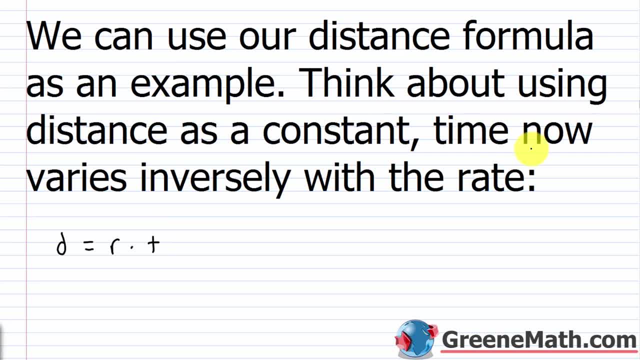 I have think about using distance as a constant. Time now varies inversely with the rate. So let me just show you this real quick: If I have y equals k over x, I can make this look like this. Remember, I'm saying that. 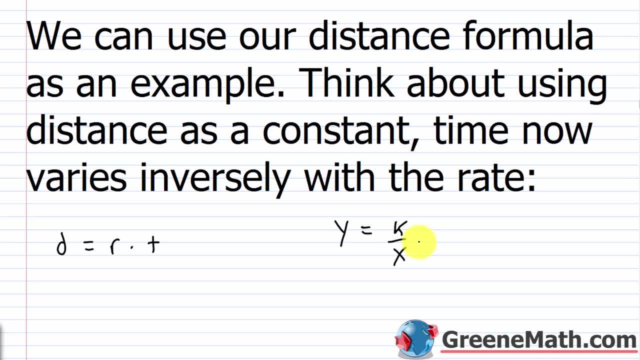 time varies inversely with rate. So my time okay is going to be y. So what I want to do is get time by itself. So divide both sides by r And what I'll have is time is equal to distance over rate. 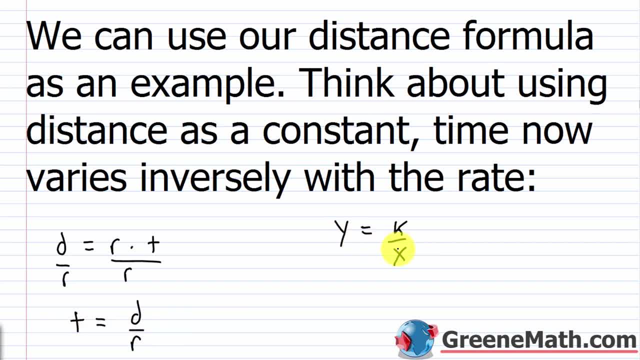 Now, time varies inversely with r, just like y varies inversely with x. Remember, we said that distance was going to be constant, right? So distance is in the numerator there, just like k is here, And you can think about an easy example of this. 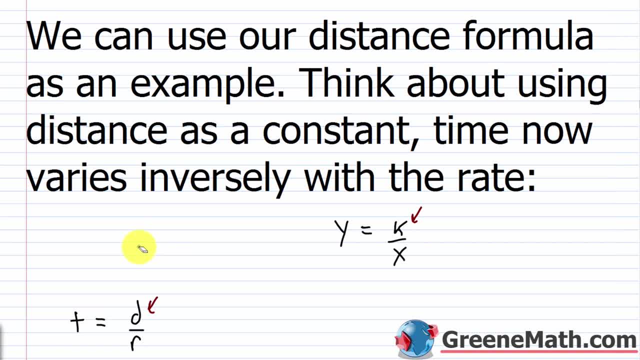 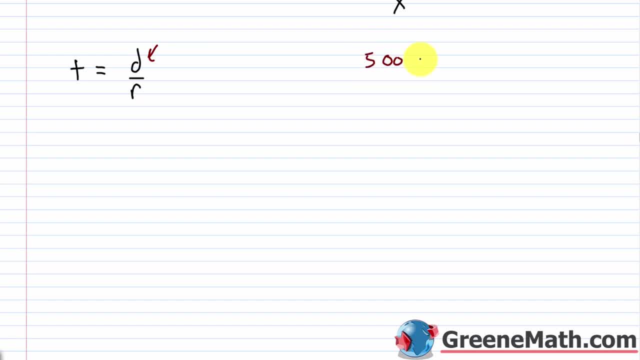 Let me kind of get a little room going here. If I think about going on a trip, let's say the trip is 500 miles, So it's 500 miles, So time equals. we'll just put 500 up here In the denominator. we have our rate of speed. 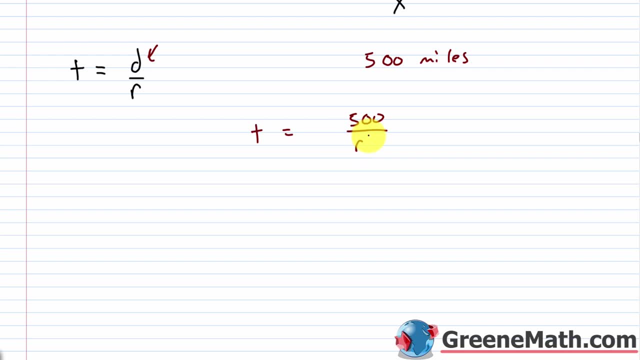 Does it make sense that this varies inversely time with rate? Yes, it does. If I increase my rate, my time is going to decrease. If I decrease my rate, my time is going to increase. Let's give you an example. 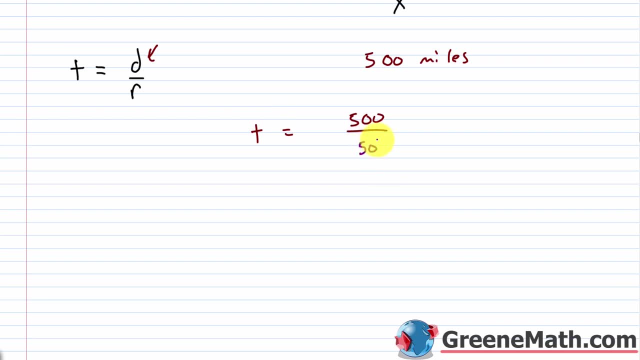 Let's say I decide to drive 50 miles per hour. So 500 divided by 50 would give me 10.. So that means that my destination took 10 hours to get to. If I increase my rate of speed, let's say I double it. 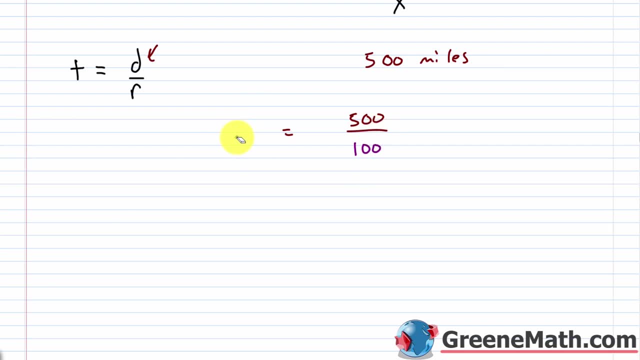 Let's say I go 100 miles an hour. Well, now my time is going to decrease. It goes from 10 to 5.. So we can see, with inverse variation, as I increase the rate, my time decreased. Now, if I decrease the rate, 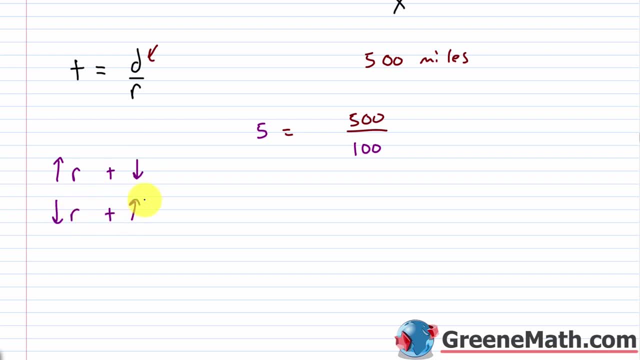 my time will increase. So they're inverse: Bring one up, the other. falls With direct variation: bring one up, the other goes up. Bring one down, the other goes down. Inverse: one goes up, one goes down. 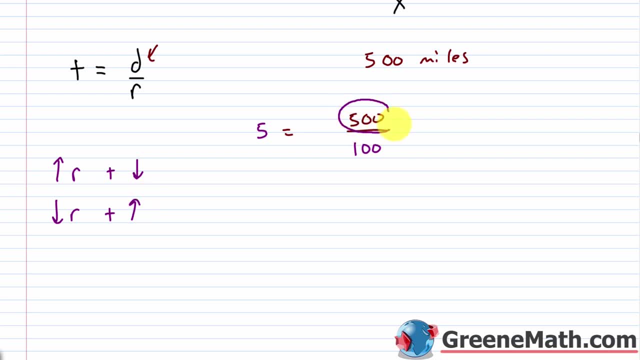 Now I should note that this is all reliant on this, the constant being positive. So you've got to note that. But if I was to, let's say, go to a slow speed, like, let's say, 25 miles an hour, 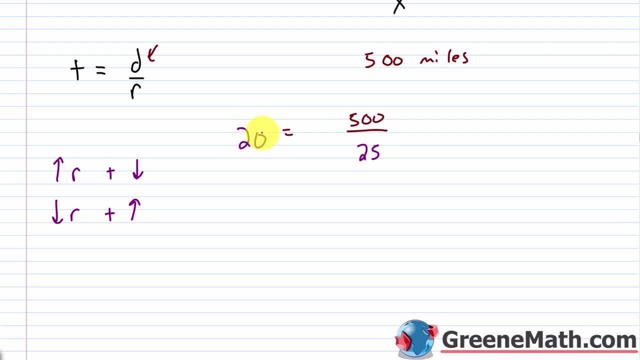 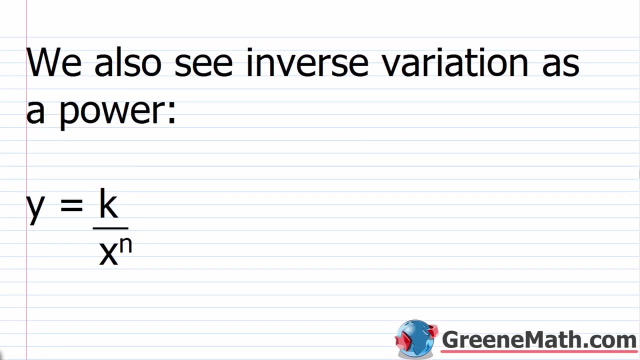 well, now it's going to take me 20 hours to get to my destination. So as I decrease the rate of speed, the time went up. Additionally, we will also see inverse variation as a power, So you might see: y equals k over x to the nth power. 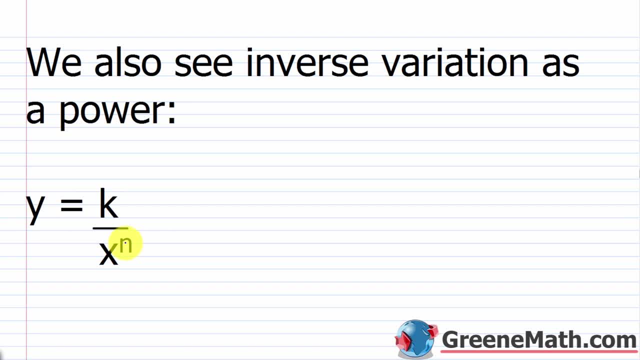 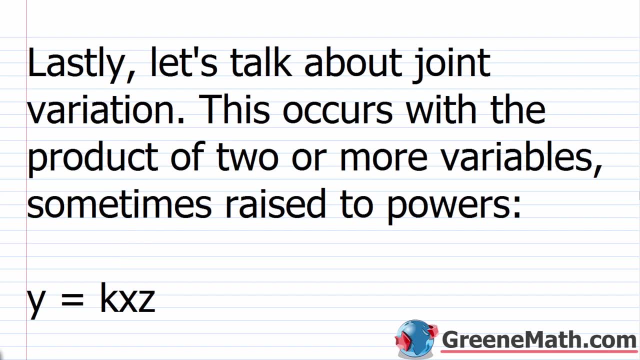 So, with direct variation as a power and inverse variation as a power, the only difference is your variable x is raised to some power. The formula is the same. other than that, Alright. so the last thing I want to talk about is joint variation. 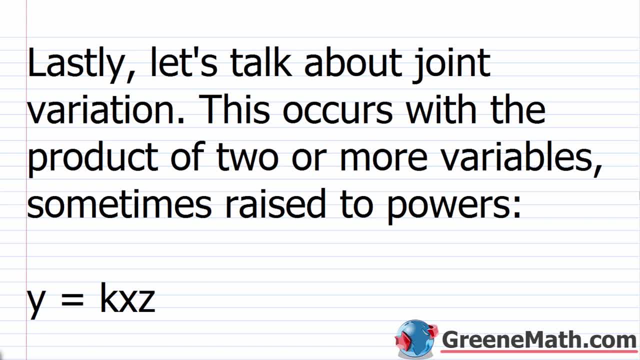 And we really didn't cover this in Algebra 1.. It's no more difficult, It's just a little bit more tedious. So this occurs with the product of two or more variables, all times raised to powers, So, as an example, y varies directly with x and z. 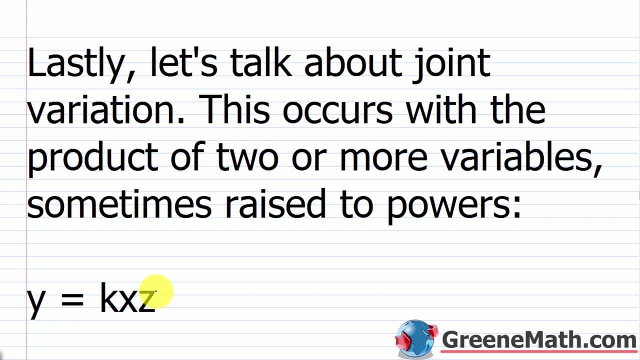 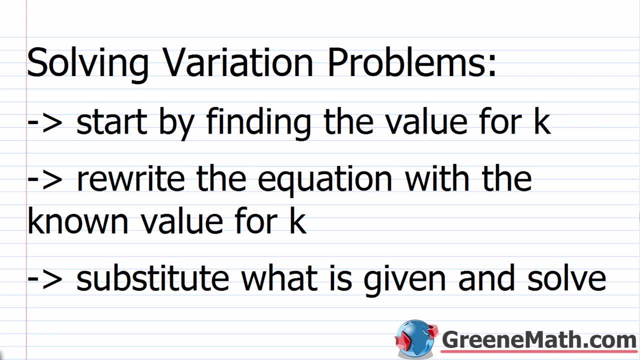 if there is a constant k, such that y equals k times x times z. Alright, so now that we understand the basics of variation, I want to talk about how to solve the variation problems that we're going to get. They're very, very, very easy. 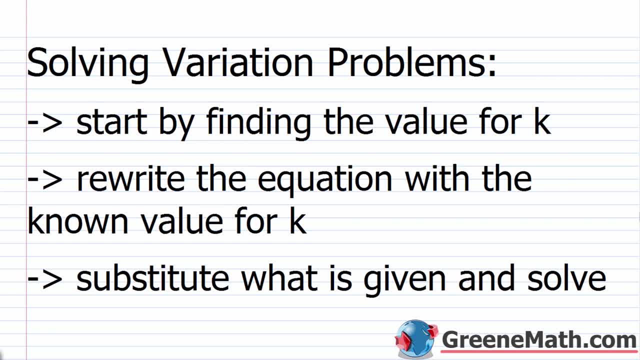 This is one of the easiest sections in all of Algebra, So just follow this procedure to the letter. You're going to be good to go. So you want to start by finding the value for k. The value for k doesn't change, So they'll give you an opening scenario. 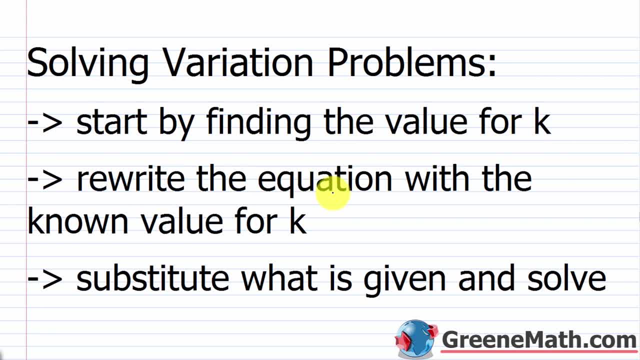 that allows you to find k. Then what you want to do is you want to rewrite the equation with the known value of k, You're going to substitute what is given in the second scenario and then you're going to solve. So write these steps down. 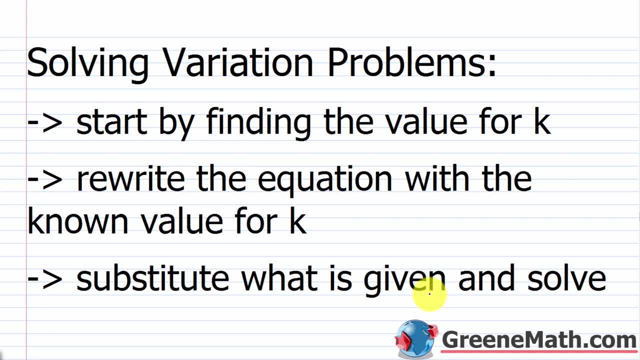 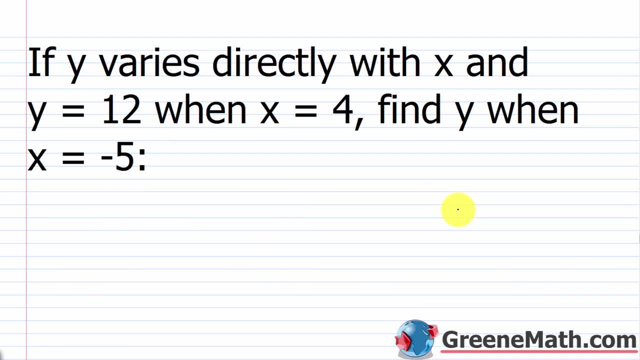 Pause the video And we're going to use them through our problems, And when you get to your textbook problems, you're going to fly right through them. They're very, very easy, Alright. so let's look at the first problem. 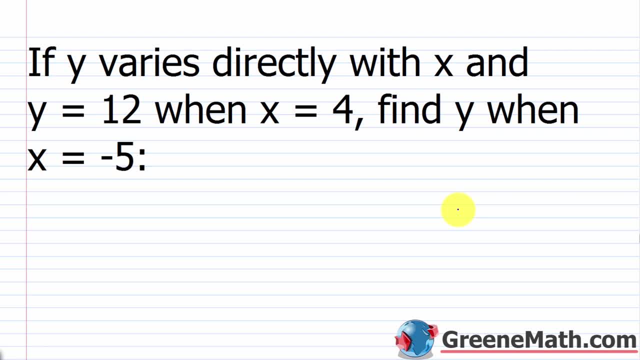 Y equals 12 when x equals. 4. Find y when x equals negative. 5. Go ahead and write out your equation. Y varies directly with x, So y equals kx. Now, what am I given? to start, I'm given that y equals 12. 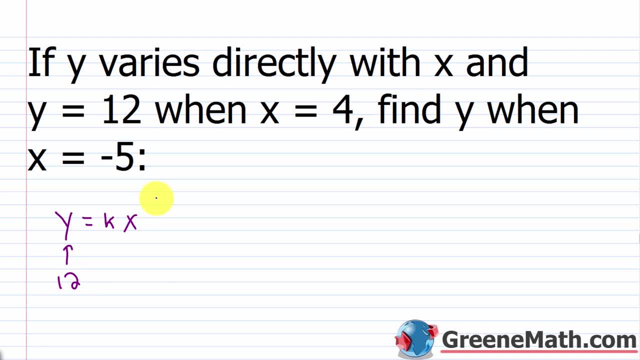 so y equals 12 when x equals 4.. So if I plug those two things in, I can find the value of k. Now one quick note. I can tell you that algebraically we can find k before we even start by dividing the value of k. 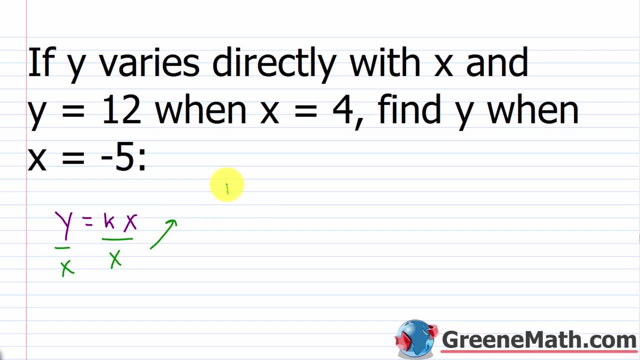 by dividing both sides by x. So this means that k is equal to y over x. So I can just plug into that and kind of skip a step. I can say: well, to find k, y would be 12 and x would be 4.. 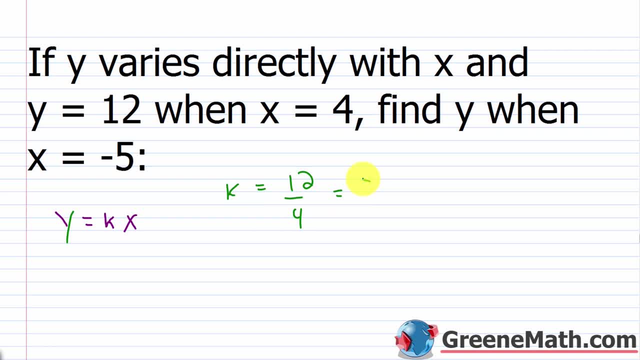 So I know that k is 12 over 4 or 3.. Now traditionally we just plug it in here and say y is 12, x is 4, and I go through an extra step and say 12 equals 4k. Then I divide both. 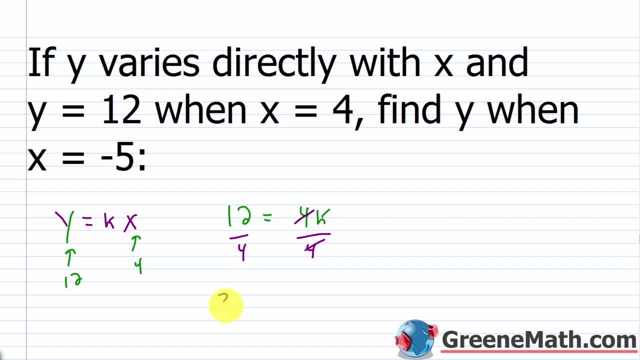 sides by 4.. This cancels and I get 3 equals k or k equals 3.. Whatever you want to do, whatever you're more comfortable with, but just know that k is always going to be equal to y divided by x, So k. 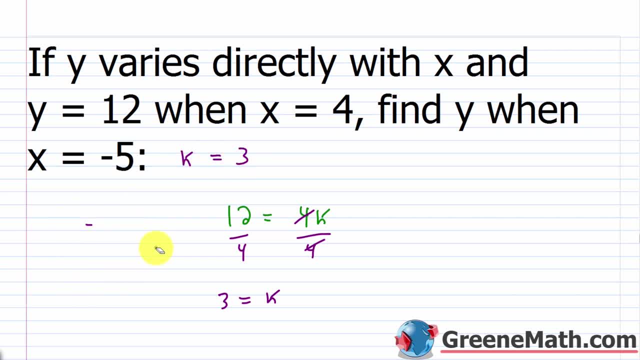 is equal to 3.. So now that we have that information, we're pretty much good to go. We just solve what they want us to solve. We're just going to find y when x equals negative 5. So y is equal to. 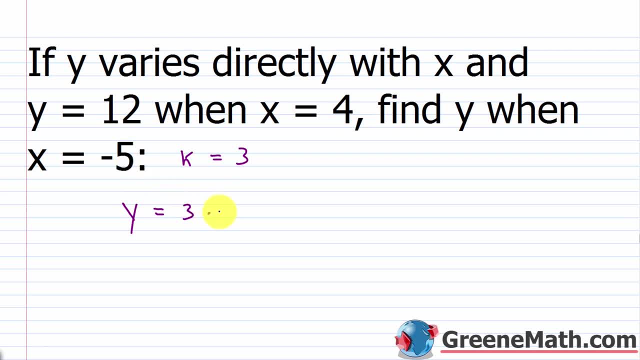 k, which we know is 3, times x, which we know is negative 5.. 3 times negative 5 is negative 15.. So we found y when x equals negative 5.. When x equals negative 5, y is negative 15.. 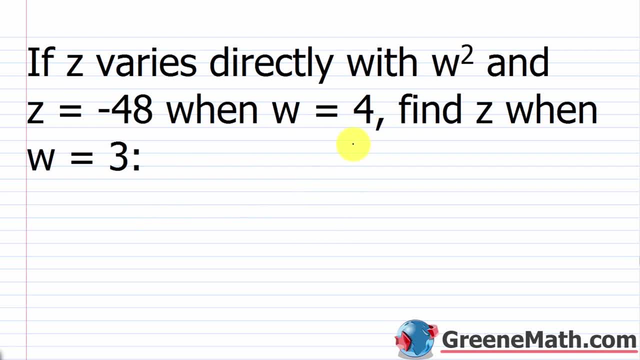 So we're done. So you saw how easy that was. If you didn't take Algebra 1 and you were kind of worried about these problems. don't be, They're very, very easy. So if z varies directly with w squared and, 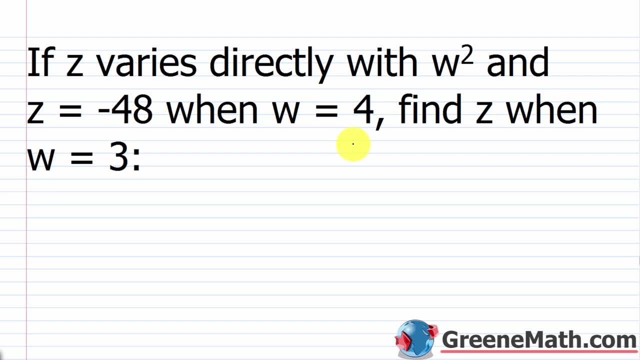 z equals negative 48, when w equals 4, and z when w equals 3.. So this is one thing that really trips up students. when you start changing letters around, They're like: what's z and w doing here? It should be y and x. 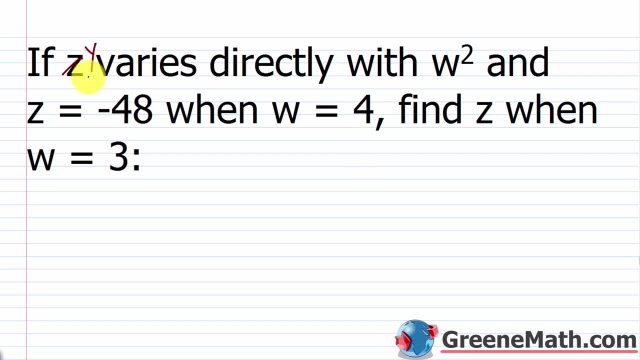 Cross things out. if you have to Say, okay, if y varies directly with x squared, what would that look like? It would be: y equals k times x squared. Or we could say that k is equal to: if I divide both sides by x squared. 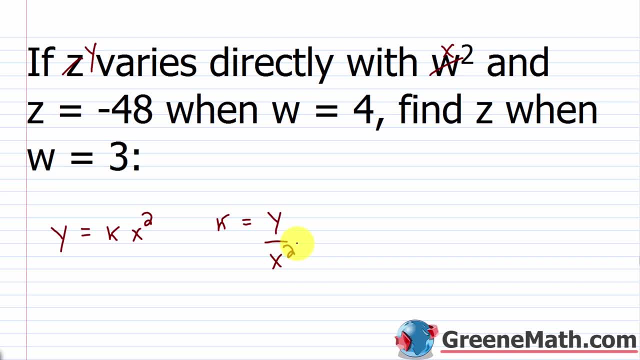 y over x squared. Here's the kicker. I can just erase this now and I can substitute a z for y And I can substitute a w for x. So this is z and this is w. If you do that a few times, you're going to get it. 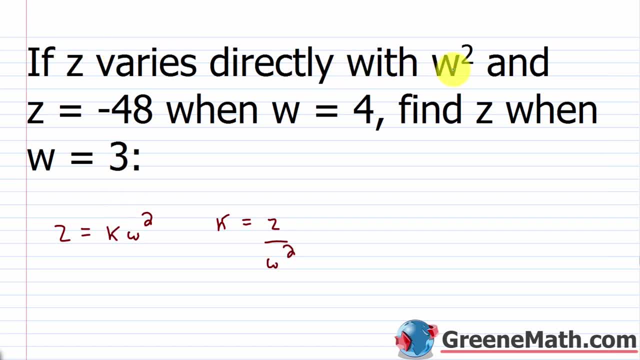 z is what varies directly with w squared. So z is equal to k times w squared. You replace it a few times and you're going to get it. It's kind of obvious, but I realize when you first see different letters it can really throw you for a loop. 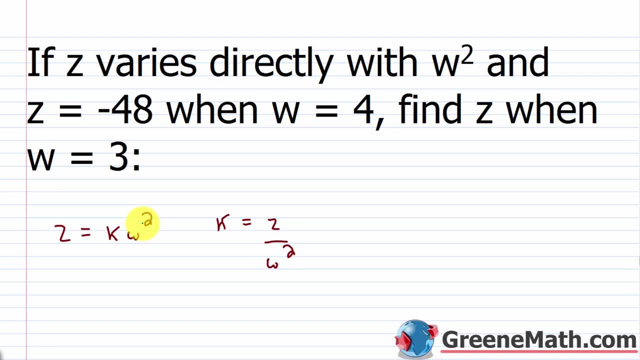 So it tells us that z equals negative 48. So I can plug in a negative 48 here When w equals 4. So 4 is going to be squared, So negative 48 over 4 squared. 4 squared is 16.. 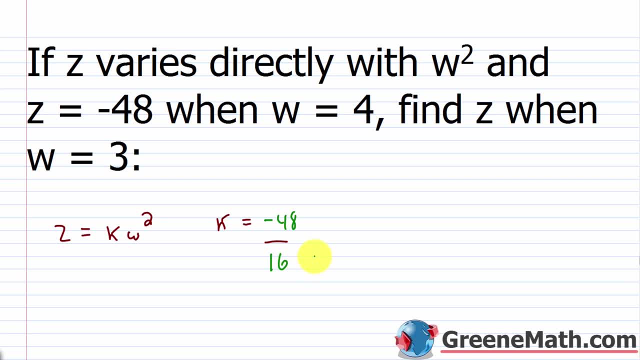 Negative 48 over 16 is negative 3.. So k will equal negative 3.. k equals negative 3.. So now they want us to find z when w equals 3.. So all I want to do is say z is equal to, k is negative 3,. 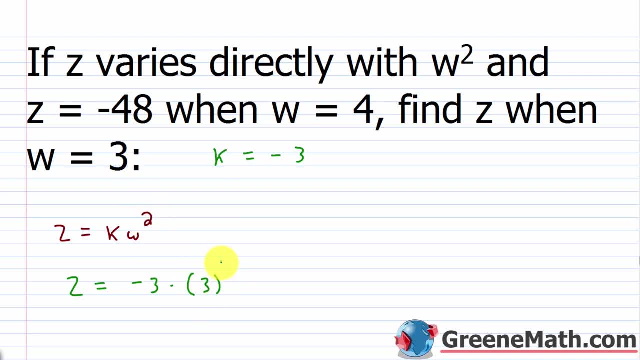 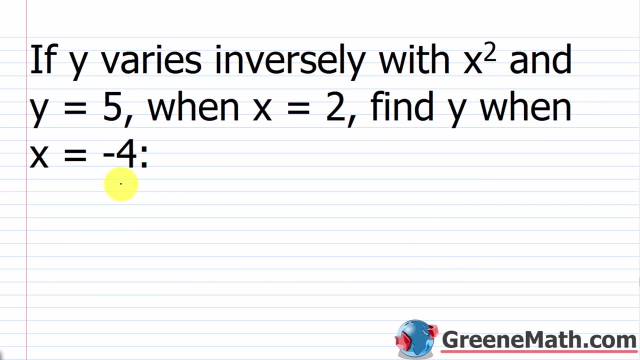 w is 3.. So we'd have 3 squared. So 3 squared is 9.. You'd have negative 3 times 9.. That's negative 27.. So z is going to be negative 27 when w equals 3.. Alright, let's take a look at another one. 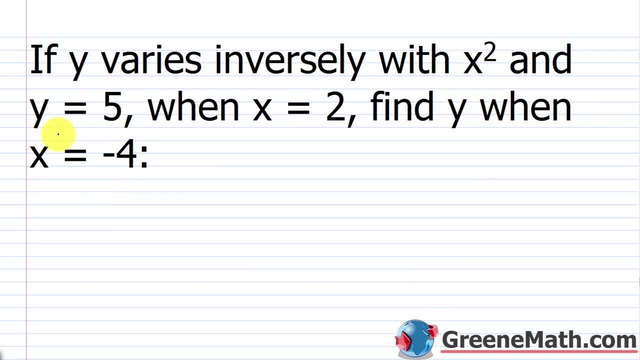 If y varies inversely, with x squared, and y equals 5 when x equals 2, we want to find y when x equals negative 4.. So we think about inverse variation. It's y equals k over x. Now, in this particular case, 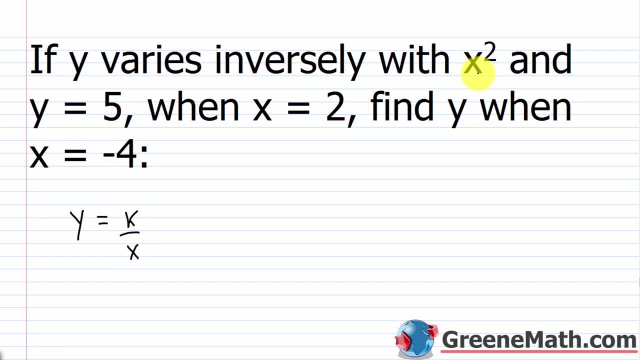 y varies inversely with x squared, So this would just be x squared here. That's the only difference. So now, how would I get k in this case? Well, I could multiply both sides by x squared, And this would cancel with this. 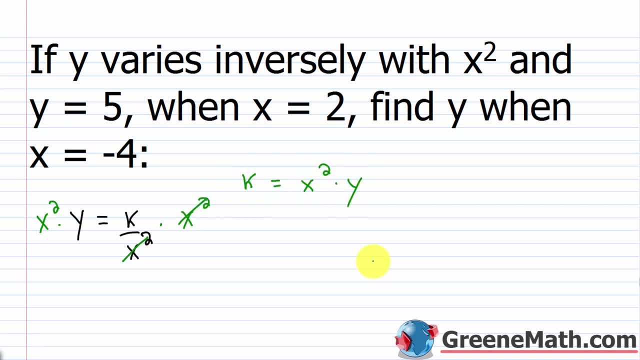 So we could say that k is equal to x squared times y. So, knowing that, let's plug in and get k. We know that y equals 5 when x is 2.. So y is 5 when x is 2.. So k will be equal to. 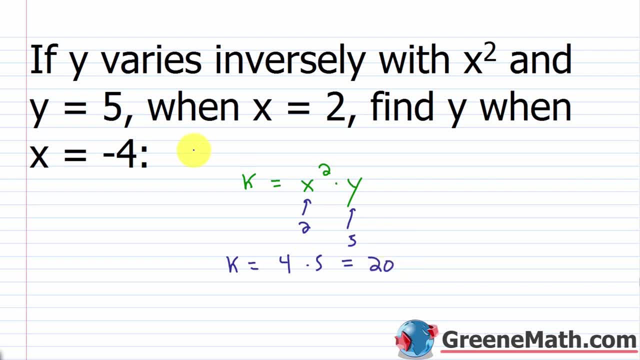 2 squared is 4 times 5, so that's 20.. So k is equal to 20.. Okay, Let's erase all this. Let's go back to that original equation: y equals k over x squared. So find y when x equals. 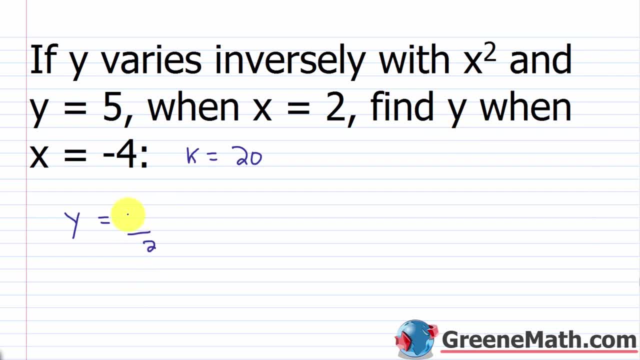 4.. So all I've got to do is plug in a 20 here and a negative 4 inside a parenthesis here, Because negative 4 is to be squared. So negative 4 times negative 4 is 16.. You think about canceling common? 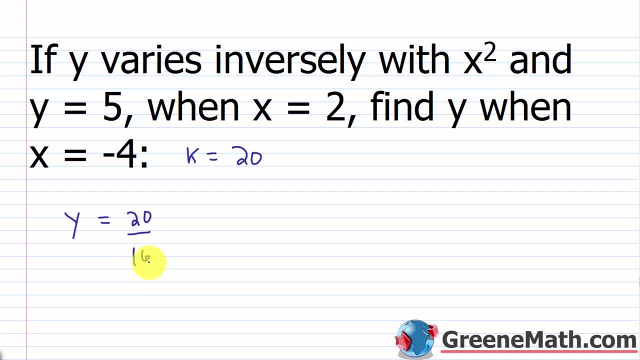 factors here. So 20 and 16 share a common factor of 4.. 20 divided by 4 is 5.. 16 divided by 4 is 4.. So basically, y would equal 5 fourths or 1.25. 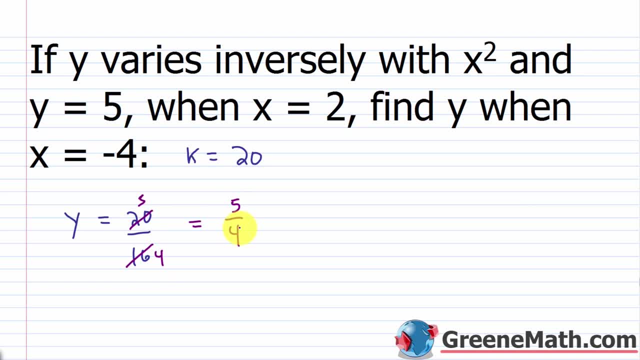 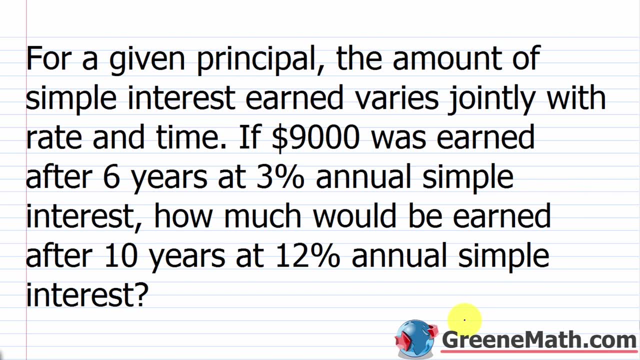 when x is equal to negative 4.. Alright, let's take a look at a few word problems here. We'll just kind of wrap this up. So for a given principle, the amount of simple interest earned varies jointly with rate and time. If $9,000 was earned, 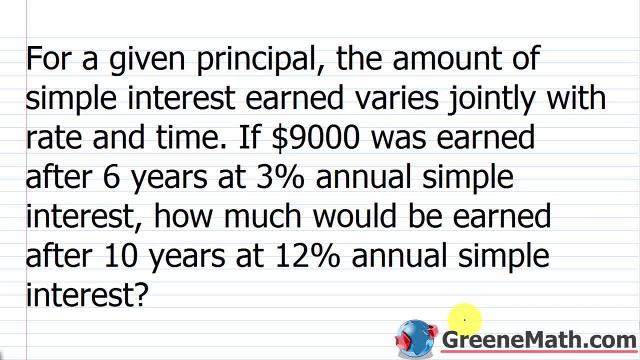 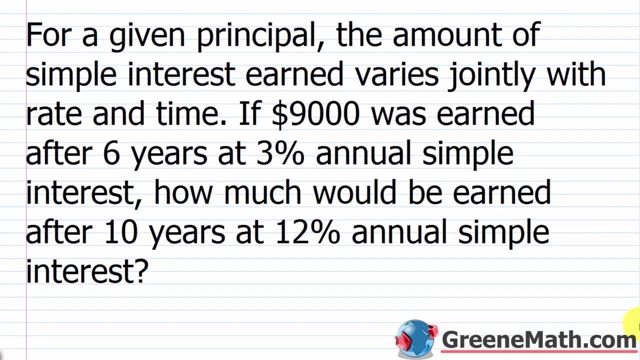 after 6 years at 3% annual simple interest, how much would be earned after 10 years at 12% annual simple interest? So think about this step by step. The first thing is, most of you already know the simple interest formula. It's i is equal to. 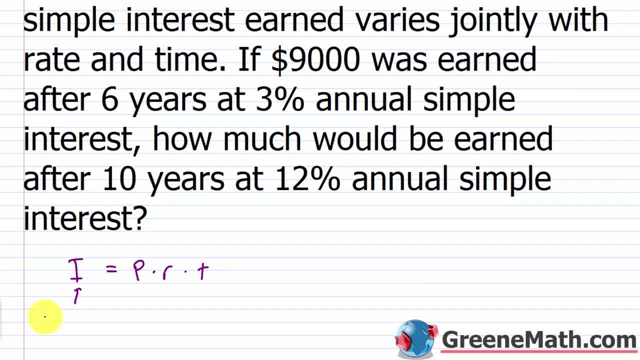 p times r times t. So i is simple: interest earned: p is the principle or the amount that is invested, r is the rate, t is the time and generally this is in years. Now, what are we given here? It tells us that for a 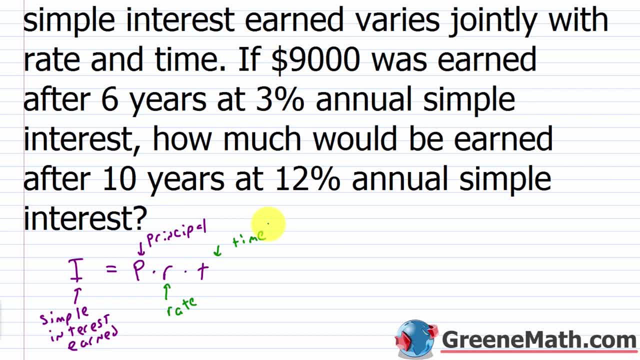 given principle. that means the principle is set. it's your constant of variation. So this guy right here is like your k. So if I had y equals k times x times z, k would be the constant of variation. That's p in this case. 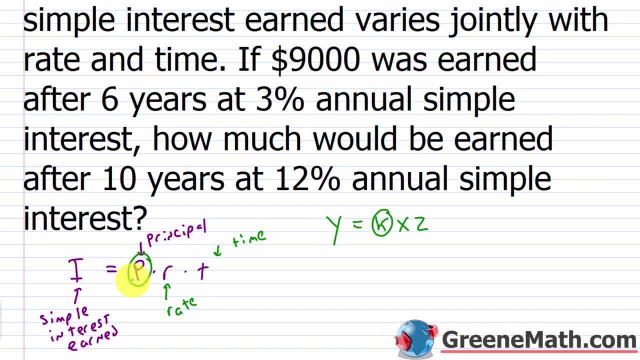 It does not change. So then the amount of simple interest earned varies jointly. So this is the simple interest earned, and it varies jointly with rate and time. So here x and z represent rate and time, y represents simple interest earned. So once we can relate it to our generic 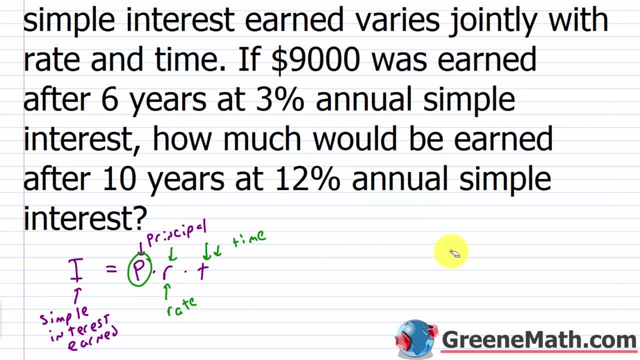 formula. we pretty much understand what's going on. So it tells me that if $9,000 was earned, okay, so that's the simple interest earned. so $9,000 after 6 years. so time is 6- at 3% annual simple interest. 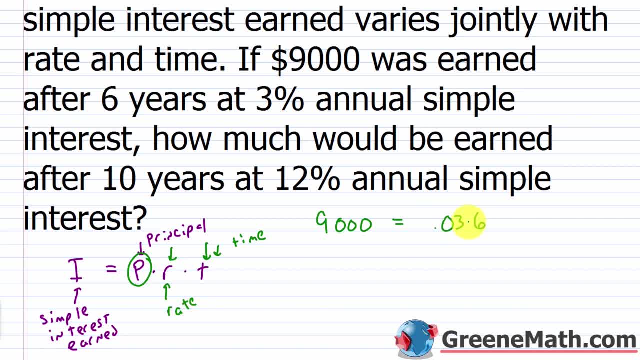 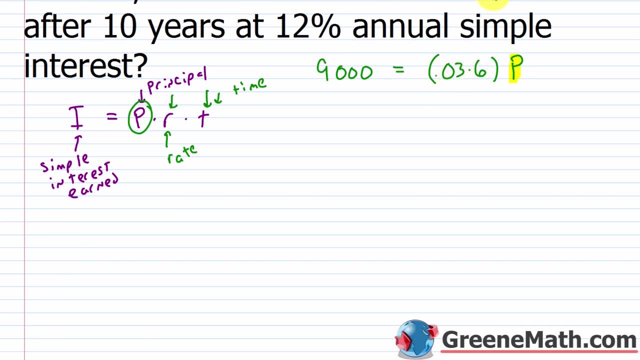 so the rate is .03. So I multiply these two together and realize I have that constant amount. the principle and my goal right now is to find that. So let's scroll down and get some room going. .03 times 6 would be what? Well, 3 times 6 is 18. 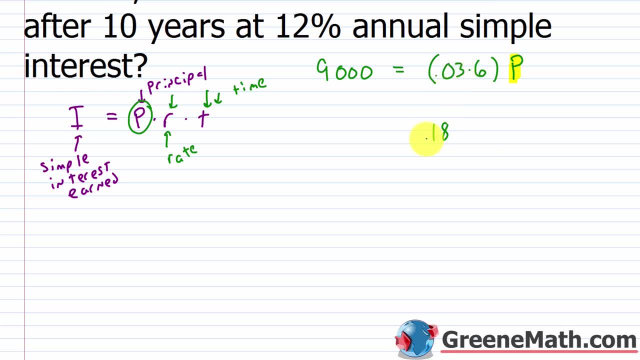 you have 2 decimal places between the factors, so this would be .18 times p and this equals 9,000. so let's divide each side by .18 and that's going to give me 50,000. so p is equal to 50,000. 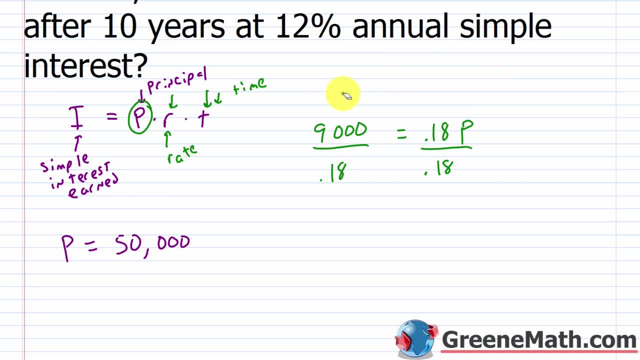 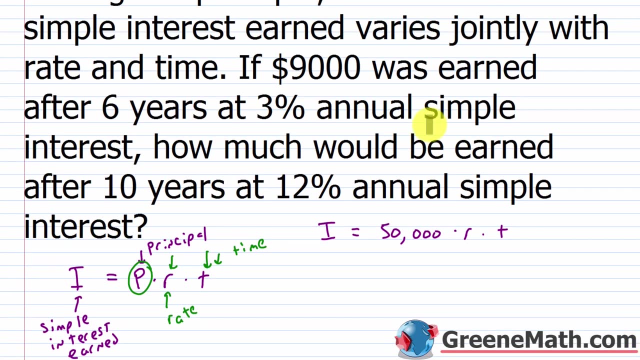 so that's the principle that is invested. that's the constant of variation. it's not going to change. I'm going to write: i is equal to 50,000, because that's my principle: times rate, times time. let's go back up. this is what we need to find. 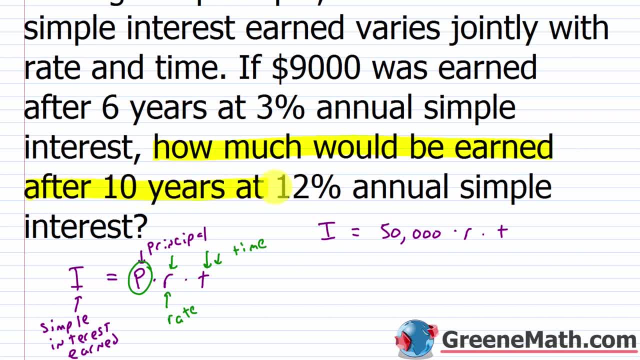 how much would be earned after 10 years at 12% annual simple interest? well, this is what I'm looking for, to find i, and I'm given the inputs. so the rate is 12%, so as a decimal that's .12, and the time is 10 years. 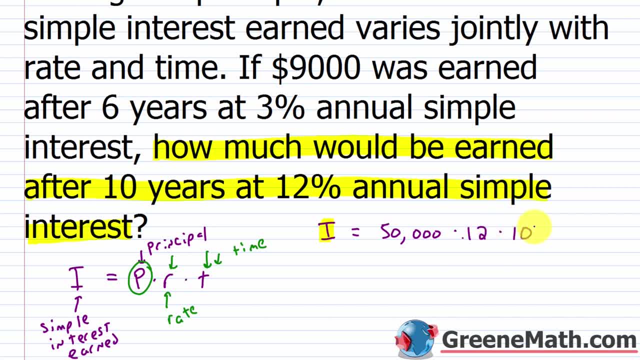 so this is just 10. so 50,000 times .12 is 6,000, and 6,000 times 10 is 60,000. so i here would equal 60,000. now we have a word problem, so let's answer it with a nice little sentence. 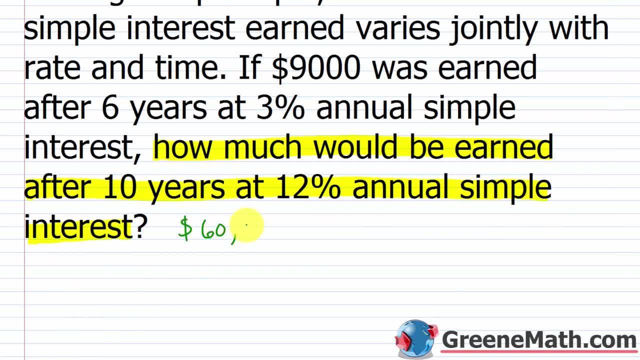 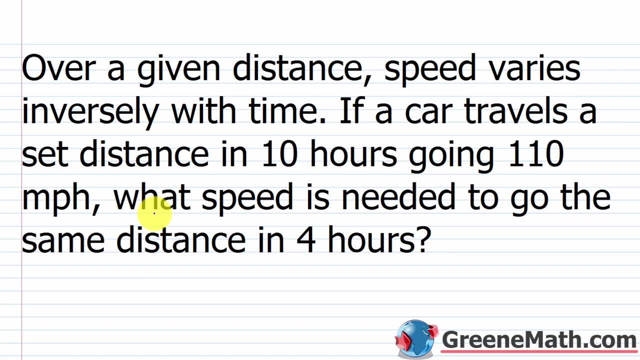 and we can say $60,000 would be earned after 10 years. alright, let's take a look at one more. so over a given distance, speed varies inversely with time. if a car travels a set distance in 10 hours, going 110 miles per hour, 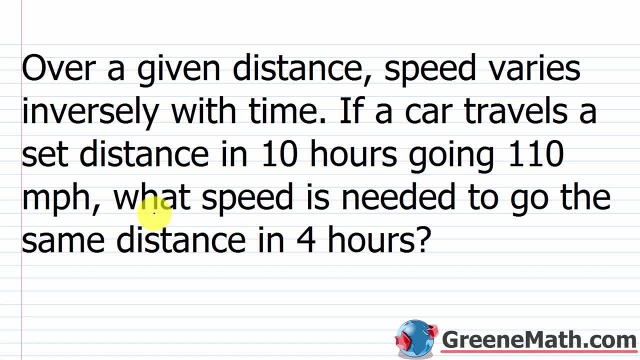 what speed is needed to go the same distance in 4 hours. so over a given distance, speed varies inversely with time. so we know our distance formula is: d equals r times t. it tells me here that speed or rate varies inversely with time. divide both sides by t. 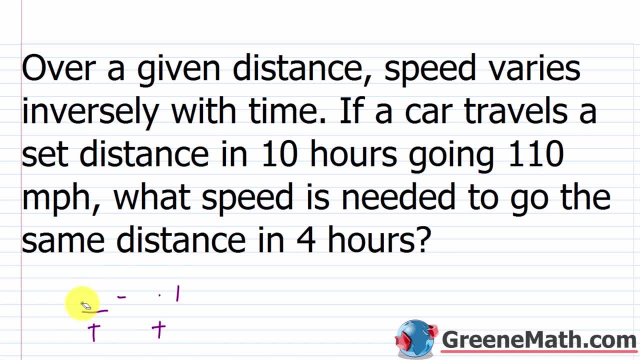 and you'll see that this cancels with this and, yeah, you'll have that. rate is equal to distance over time. so the distance is what's going to be fixed here. it's not going to change. it's a set distance. so that's my constant of variation. 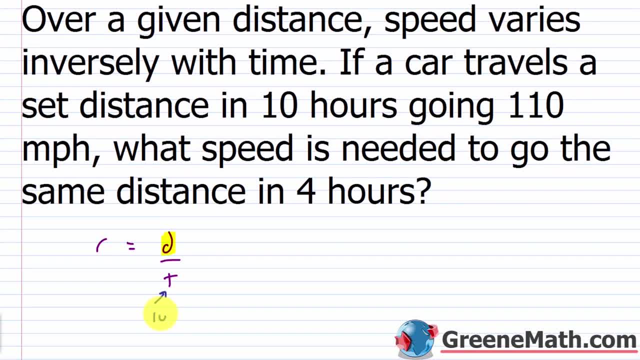 now, if a car travels a set distance in 10 hours, so the time is 10 and the rate is 110 miles per hour. so if i multiply the two together 10 times 110 is 1100, so the distance here is 1100 miles. 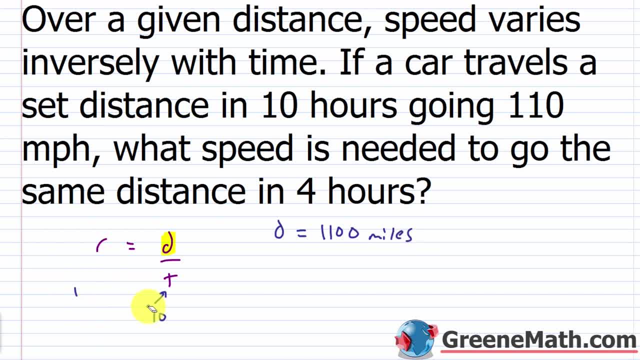 that's a constant. it's not going to change. now, if i take 1100 and i think about what else i need, what speed is needed to go the same distance in 4 hours, we'll just plug a 4 in here. just plug a 4 in here. 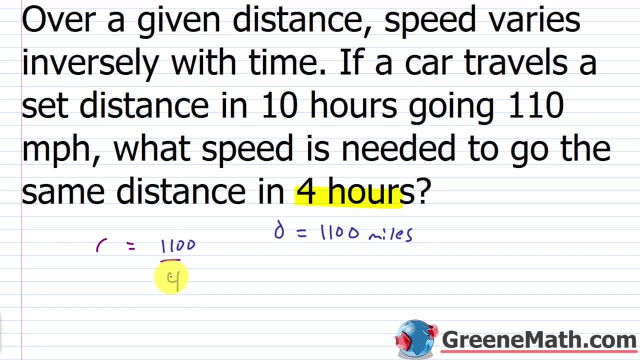 and we'll get our needed rate. so 1100 divided by 4 is 275. this is 275, so we need to go 275 miles per hour. so let's erase this and we can say that a speed of 275 miles per hour is needed. 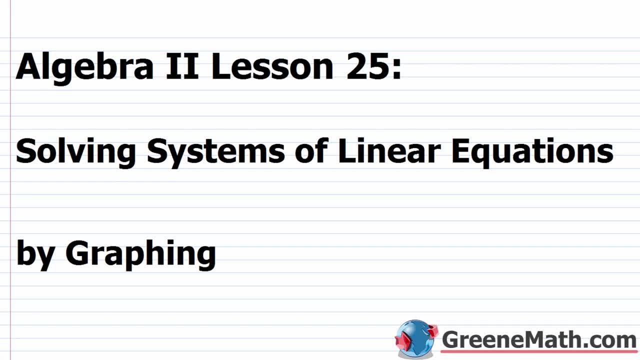 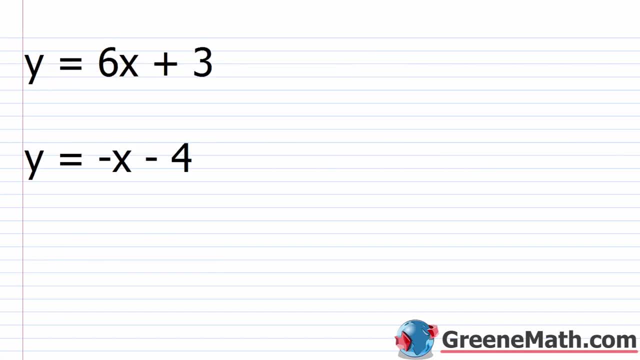 hello and welcome to algebra 2, lesson 25. in this video we're going to learn about solving systems of linear equations by graphing. so if you previously took an algebra 1 course, you're fairly familiar with how to solve a system of linear equations with graphing substitution. 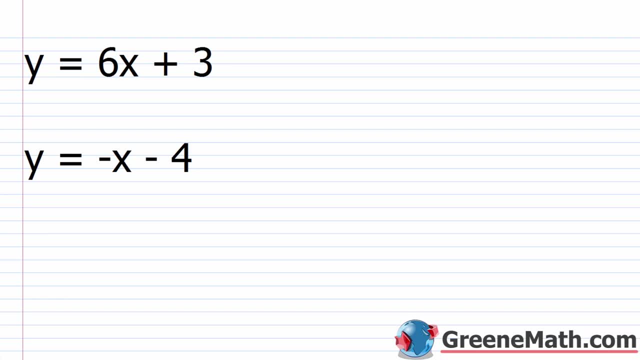 and elimination. but for those of you who haven't taken an algebra 1 course or you just never ran into this, i can tell you it's a fairly easy topic to understand. so we just start out with looking at one linear equation and two variables. i have: y equals 6x plus 3. 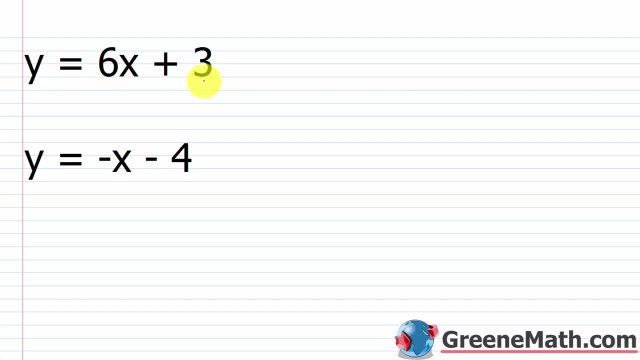 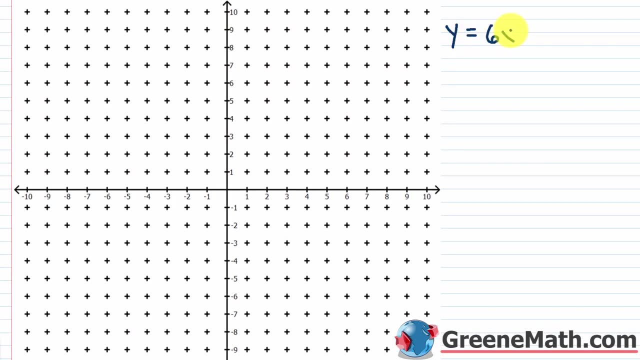 so it's a linear equation and two variables, and i can graph this on a coordinate plane. so let's just go ahead and do that real fast. so i have y equals 6x plus 3 graphically. what does that look like? well, i know, at this point it's easy. 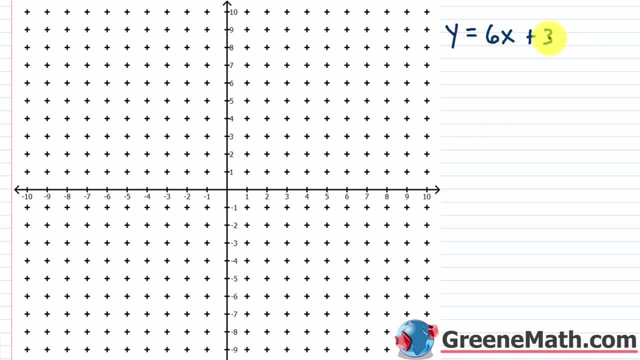 to graph something in slope intercept form. my y intercept occurs at 0 comma 3, so that's going to be right here and my slope is 6, so i will go up 6, 1, 2, 3, 4, 5, 6 to the right, 1. 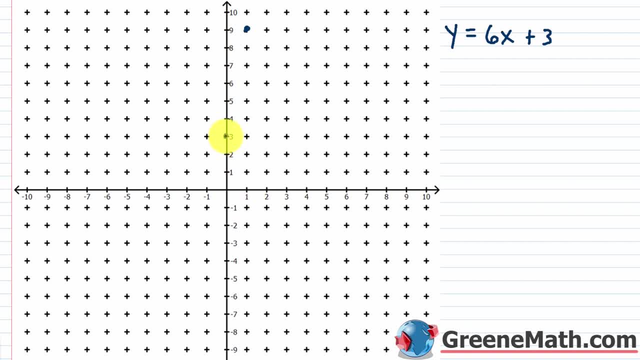 or i could go down 6. i could go down 1, 2, 3, 4, 5, 6 and go to the left one. so let's go ahead and graph this guy, ok? so this is the graph, for y equals 6x plus 3, so nothing new. 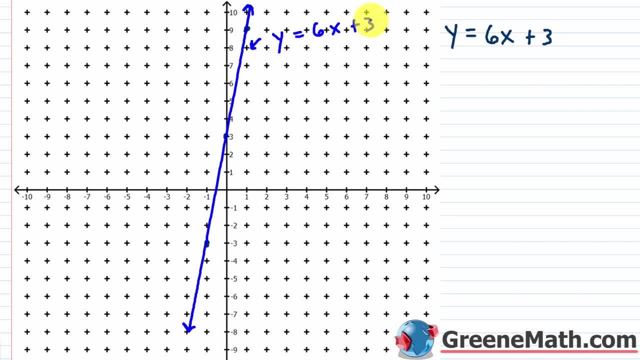 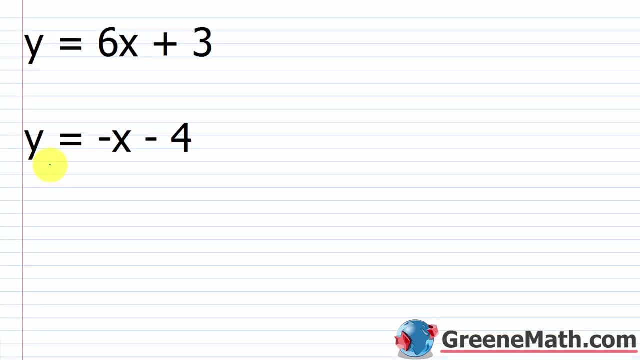 we just graphed a linear equation and two variables, no big deal. i want to go back to the previous page and i want to now take a look at this other linear equation and two variables and notice how the variables are the same: we have y, we have y, we have x. 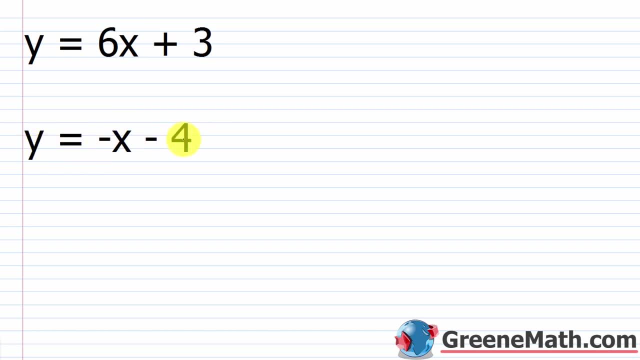 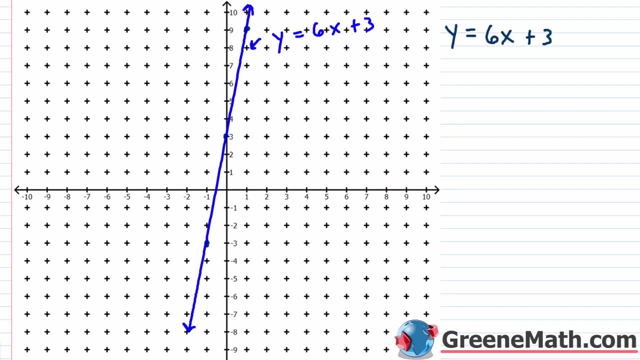 so what happens if i graph this equation on the same coordinate plane? let's take a look. so y equals negative x minus 4. so y equals negative x minus 4. so the y intercept here occurs at 0 comma, negative 4. so that's here. 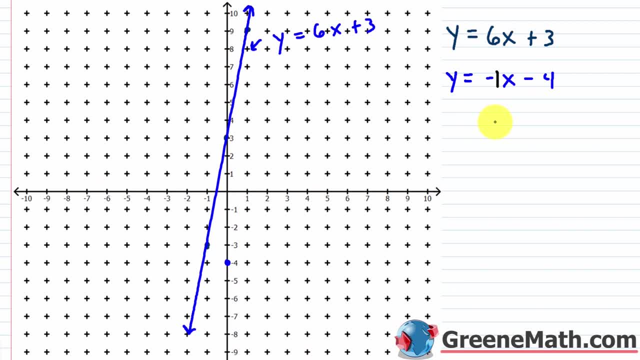 and my slope is now negative 1. right it's negative 1. so i would go down 1 to the right, 1. down 1 to the right, 1. or i could go up 1 to the left 1. up 1 to the left: 1. 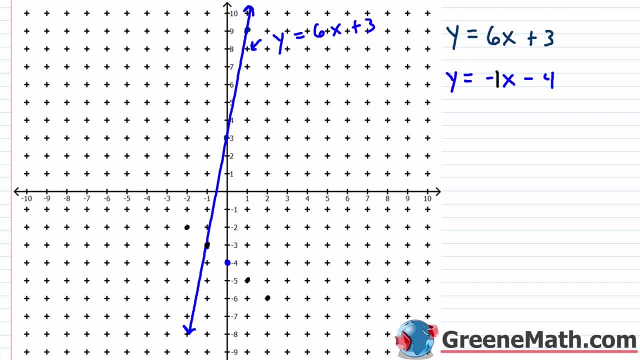 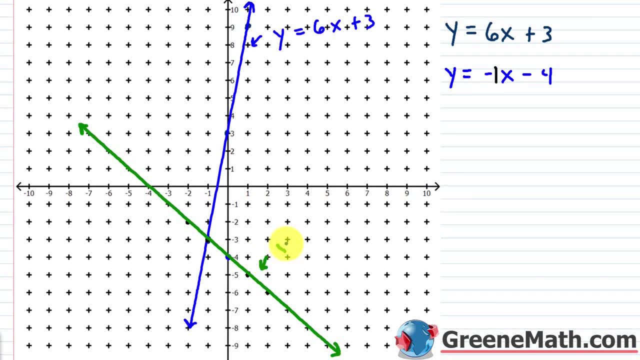 so let's go ahead and sketch this graph. so this is the graph, for y equals negative x minus 4. i want to bring your attention to something immediately. you notice that this point, right here, is a point of intersection. so that point occurs at negative 1 for the x value. 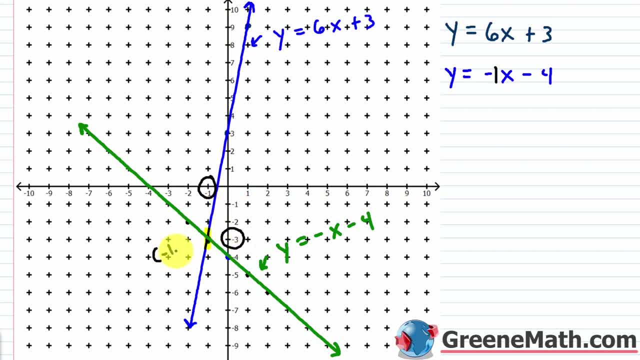 negative 3 for the y value. so this is negative 1 comma, negative 3. that point is significant because it lies on both lines, so let's think about what that means for a second. each and every point on this blue line here is a solution to: y equals 6x. 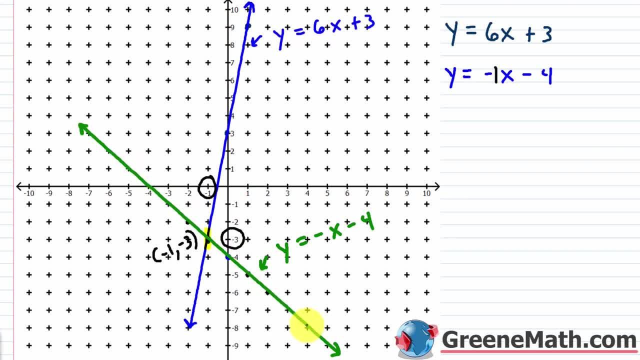 plus 3. each and every point on this green line is a solution to y equals negative x minus 4. so the point of intersection: if it lies on both lines, that means it's a solution to both of them and therefore it's a solution to our. 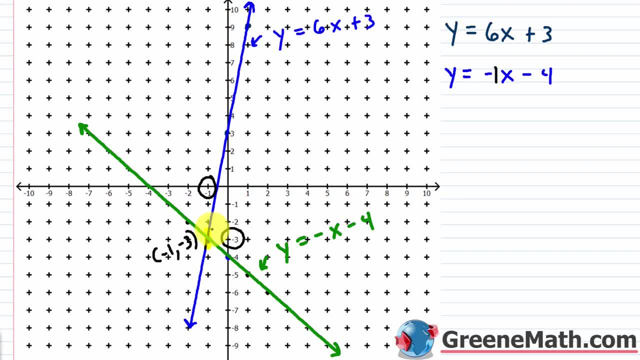 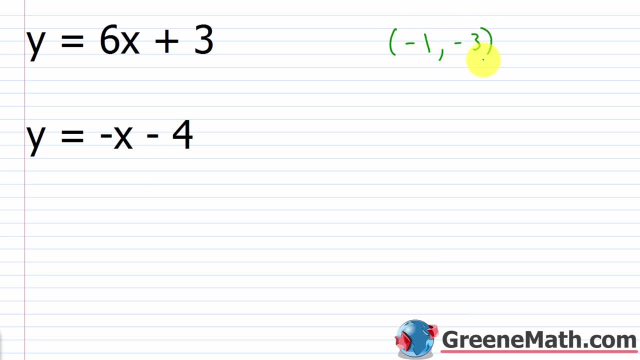 system of linear equations in two variables. so we revisit our page and we bring our ordered pair: negative 1 comma, negative 3. so these two equations, when we put them together, represent a system of linear equations. sometimes we'll say a linear system. so if i have 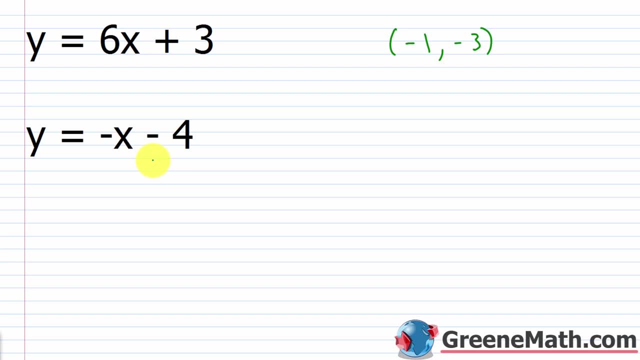 y equals 6x plus 3 and y equals negative x minus 4. my goal for a solution for a system of linear equations is to have a solution that works in both of the equations. so would this ordered pair be a solution to each equation according to our graph? 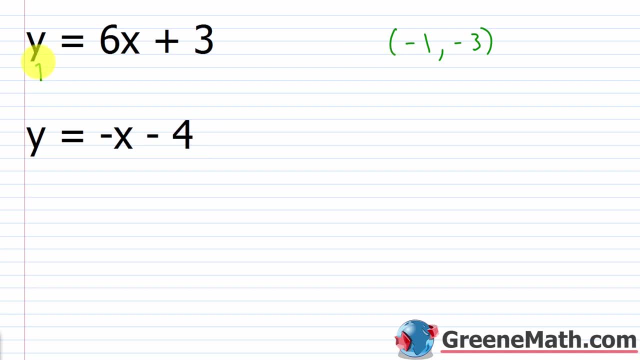 it was. let's verify. so for this one, i'm going to plug in a negative 3 for y and a negative 1 for x, and i'll see if i get a true statement i'll have. negative 3 is equal to 6 times negative 1 plus. 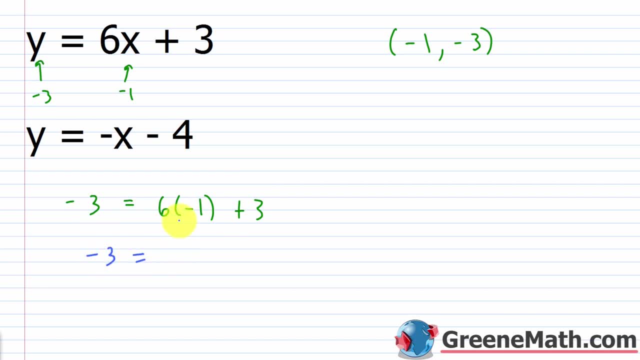 3, so i'll have: negative 3 is equal to 6 times negative. 1 is negative 6 plus 3, so then negative 6 plus 3 is negative 3, so i end up with negative 3 is equal to negative 3, so yeah, it works out. 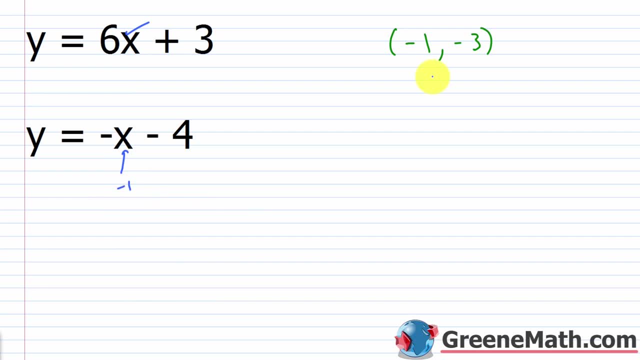 here. alright, for the next one, i'm going to plug in a negative 1 for x and i'm going to plug in a negative 3 for y. so negative 3 is equal to. you have the opposite of negative 1, so the opposite of negative 1. be careful with that sign. 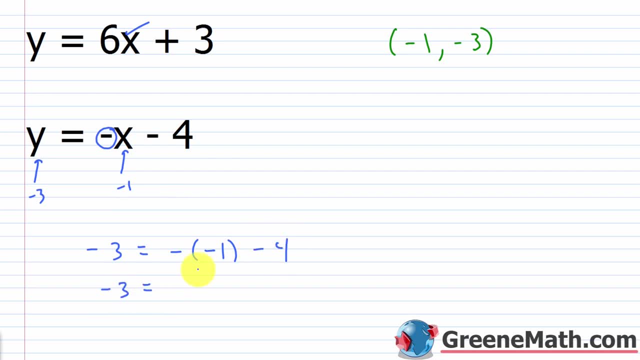 and minus 4, so negative 3 is equal to the opposite of negative. 1 is 1, so you'd have 1 minus 4. 1 minus 4 is negative 3, so you'd have negative 3 equals negative 3, so it works out here as: 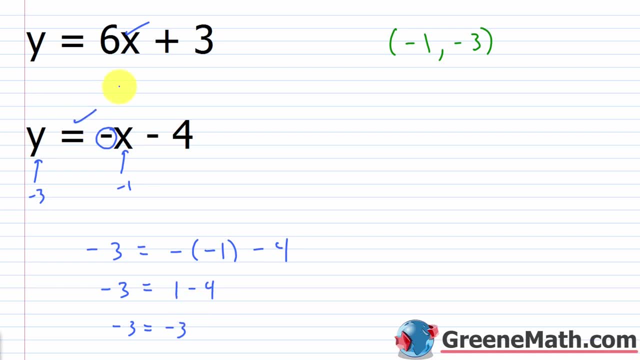 well, so we have found a solution for the system, because this solution here works in both equations. if it works in one but doesn't work in the other, it's not a solution for the system. so that's why, when we're trying to find the solution graphically, 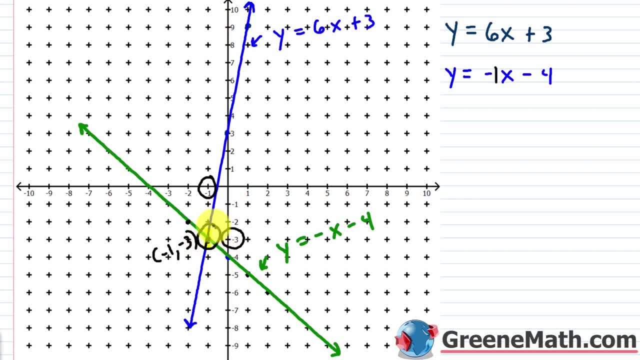 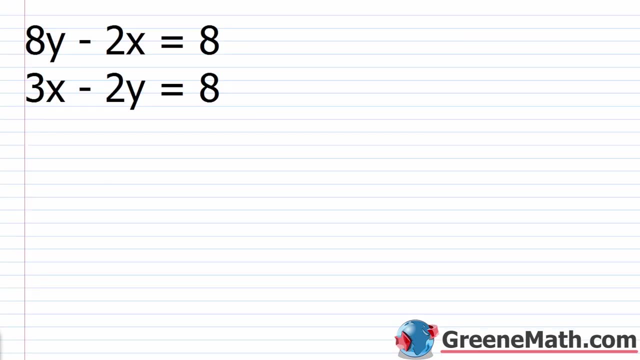 i go back to this. we look for the point of intersection, because that point lies on both lines and therefore it satisfies both equations and it's a solution for the system. alright, let's go ahead and take a look at another example. so the first one was pretty easy, because both 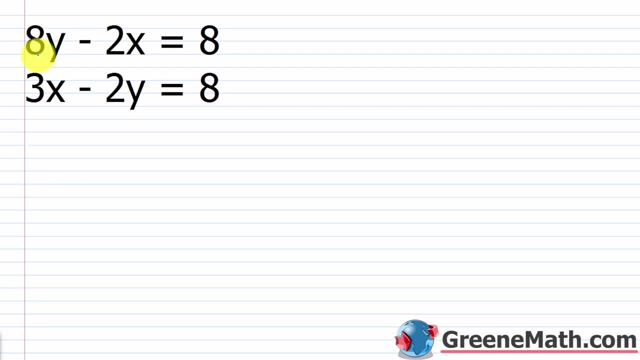 equations were solved for y. this one is going to be a little bit more tedious, so for myself, i like everything to be in slope. intercept form just makes it really easy to graph. so i'm going to solve all the equations for y. so it's going to say y equals. 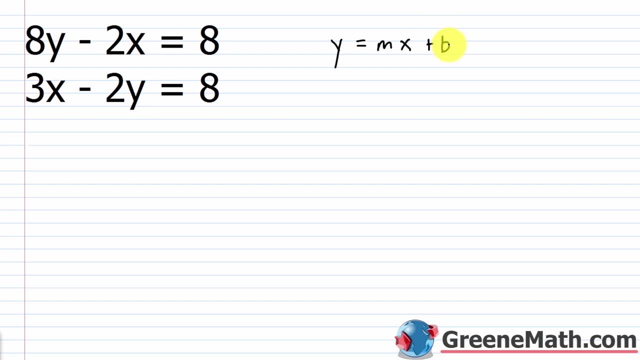 m the slope times x plus b, because then i have a point on the line and i have the slope, so it's very, very easy to graph things, alright. so let's take this guy and let's solve it for y, so 8y minus 2x. 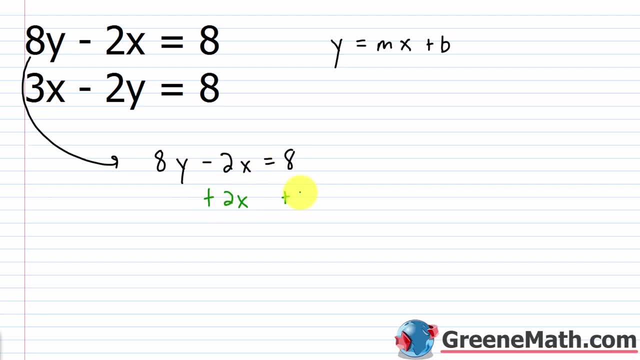 equals 8. let's go ahead and add 2x to both sides of the equation. that'll cancel. we will have: 8y is equal to 2x plus 8. divide both sides of the equation by 8 and what i'm going to have is: 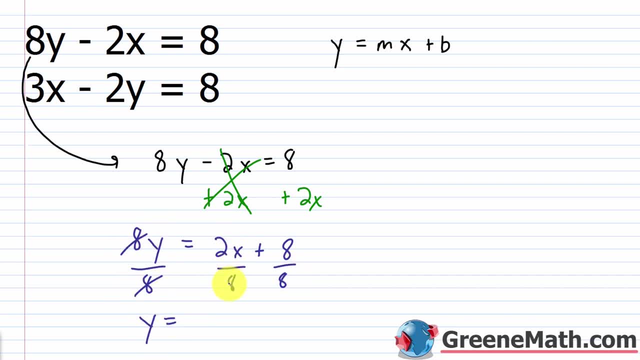 this will cancel. with this. y equals 2 over 8 is 1 fourth, so 1 fourth times x plus 8 over 8 is 1. so let's write this here. we'll write: y equals 1 fourth x plus 1. we'll just draw a little arrow to that. 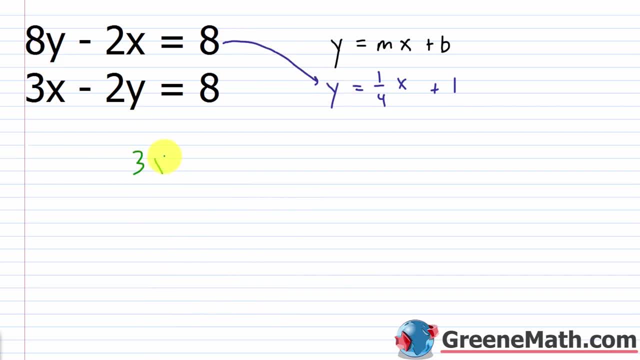 and let's erase everything. alright for this one. we'll start out with 3x minus 2y equals 8. let's subtract 3x away from each side of the equation, so we know that this is going to cancel. we'll have negative 2y. 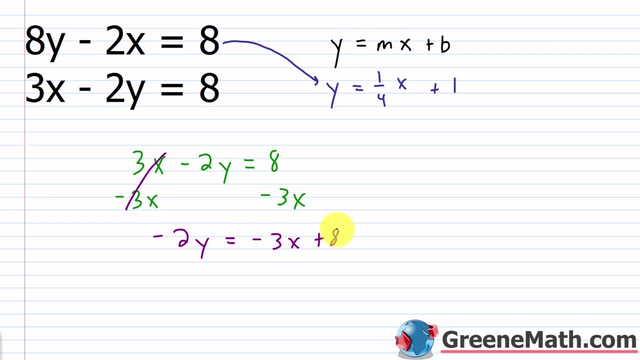 is equal to negative 3x plus 8. let's go ahead and divide both sides of the equation by negative 2, so this will cancel. y is equal to negative. 3 over negative 2 is just 3 halves times x. 8 over negative 2 is. 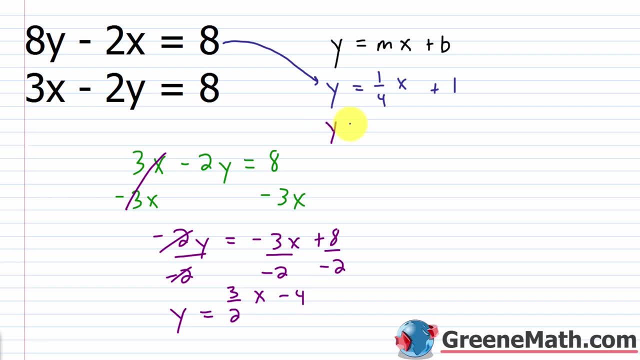 minus 4. so now we can write this one as: y equals 3 halves x minus 4. we'll drag this over here. let me erase everything now. our two equations are in slope intersection. that makes them super easy to graph. so let's go to the 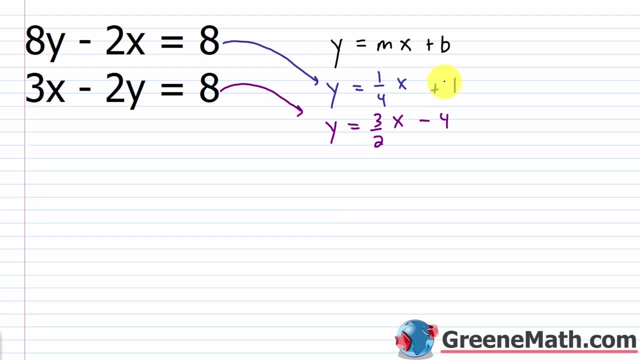 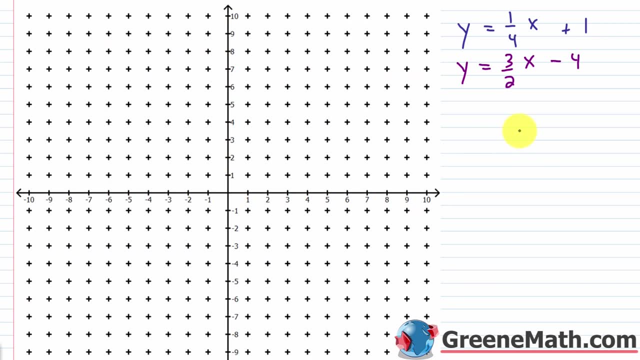 coordinate plane. we're going to graph each equation and we're going to find the point of intersection. so the point of intersection again is going to be our solution for the system. alright, so for the first equation we have: y equals 1. fourth, x plus 1. 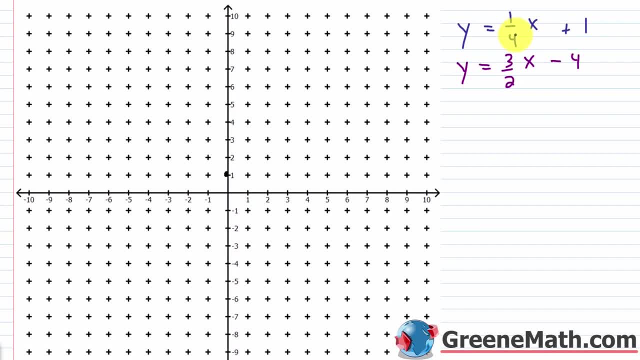 so my y intercept is at 0 comma 1 and my slope is 1, fourth. so I would go up 1 to the right, 1, 2, 3, 4. up 1 to the right, 1, 2, 3, 4. of course I could also say: 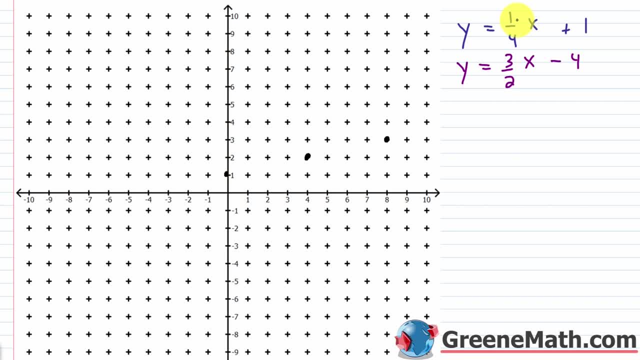 1. fourth is the same as negative 1 over negative 4. so I could start from here and I could go down 1 and to the left: 4. 1, 2, 3, 4. down 1. to the left: 1, 2, 3, 4. 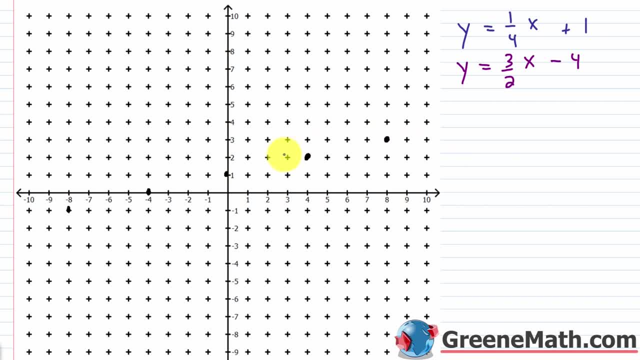 so we all know that two points make a line, but more points will help you to get a more accurate drawing, alright, so let's go ahead and sketch the graph here. alright, so this is the graph. let me go ahead and label this. of y equals 1, fourth x plus 1. 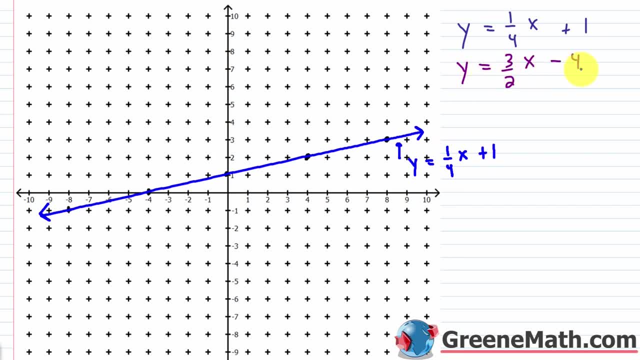 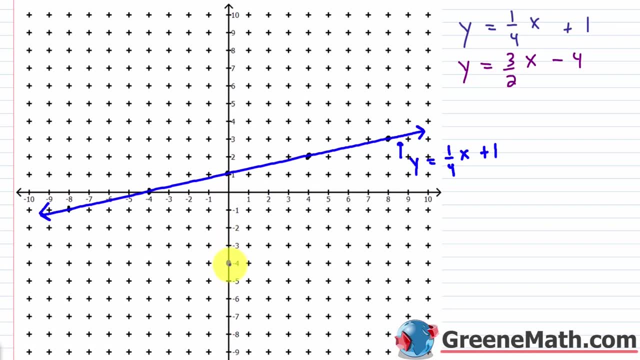 now for the other one. I have y equals 3 halves x minus 4. so the y intercept occurs at 0 comma negative 4. that's right here. the slope for this one is 3 halves. so go up 3, 1, 2, 3 to the right, 2. 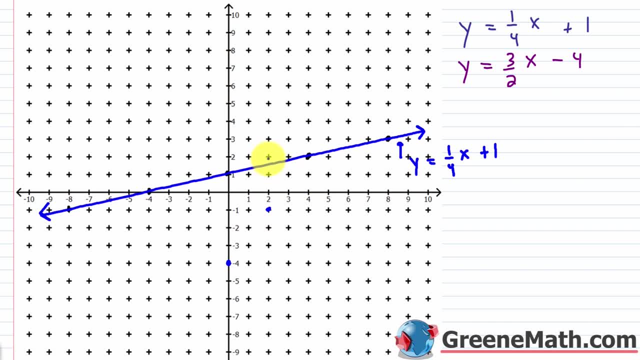 1 2. up 3 1 2, 3 to the right: 2 1 2. you can see your point of intersection there: up 3 1 2, 3 to the right, 1 2. alright, let's go ahead and graph this guy. 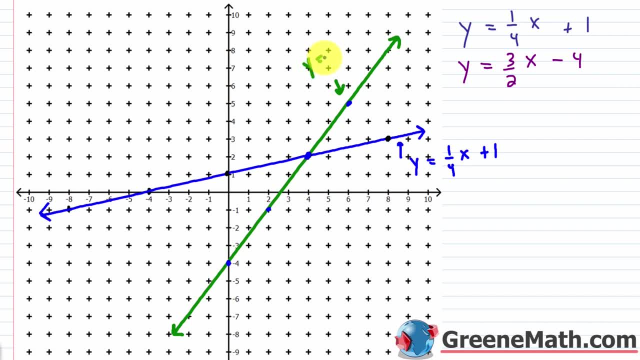 so again, this is the graph of y equals. you have 3 halves x minus 4. so the main thing here is to look for the point of intersection. that's right here. so that's where we have an x value of 4, a y value of 2. so the ordered pair. 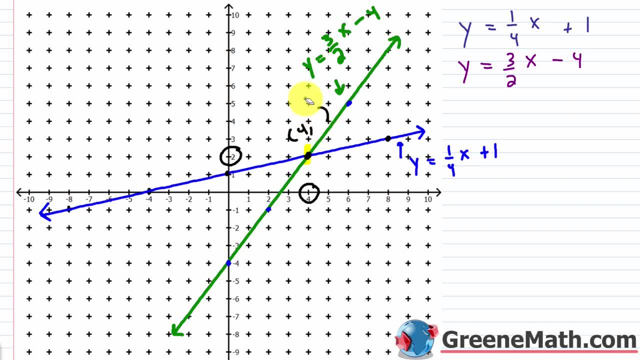 4 comma 2. and why is that significant again? well, because it lies on both lines. if a point lies on a line, that means it's a solution to that particular equation. so if this one lies on both lines, at the point of intersection, it's a. 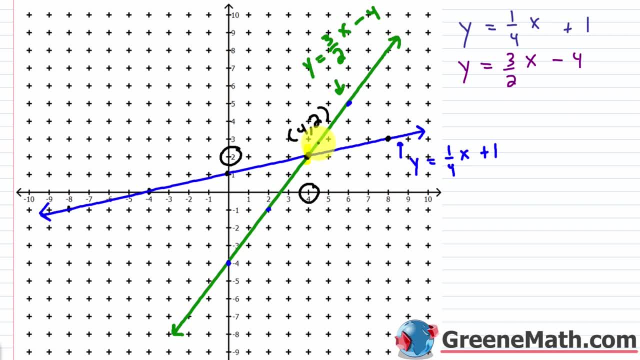 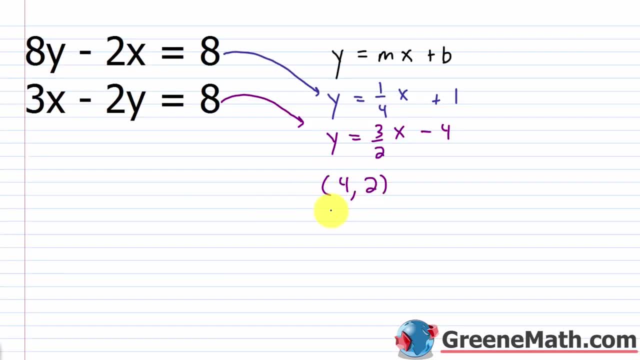 solution to both equations and therefore it's a solution to the system. so let's go back and again. our ordered pair was 4 comma 2, and we can verify this, so I'd plug in a 4 for each x and a 2 for each y. 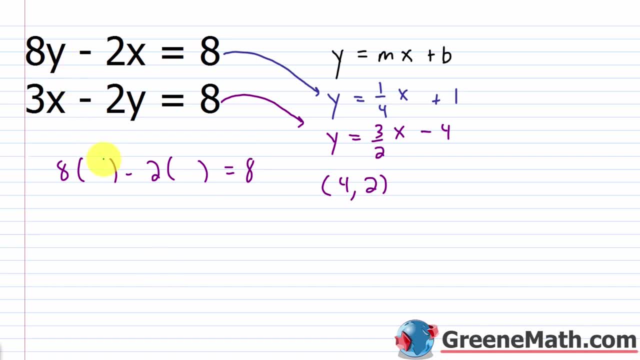 and see if the left and the right sides are equal. so for y, I'm plugging in a 2. for x, I'm plugging in a 4. 8 times 2 is 16 minus 2 times 4 is 8. 16 minus 8 is 8. 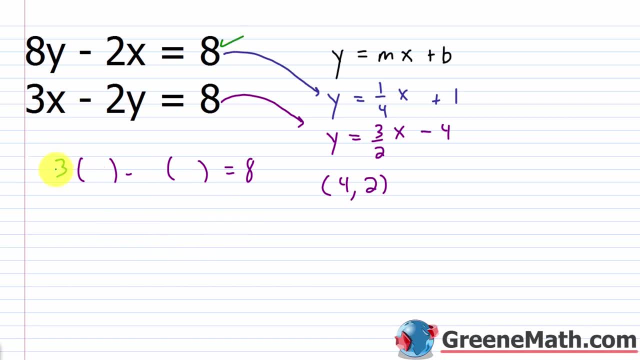 so this first one checks out for the second one. now I would have 3 times. for x, I'm plugging in a 4 minus 2 times. for y, I'm plugging in a 2 and this should equal 8. 3 times 4 is 12 minus 2 times 2 is 4. 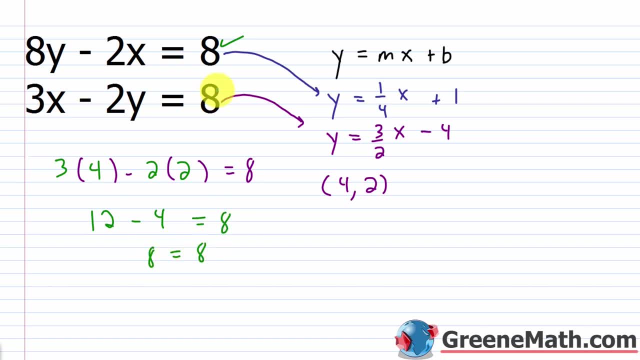 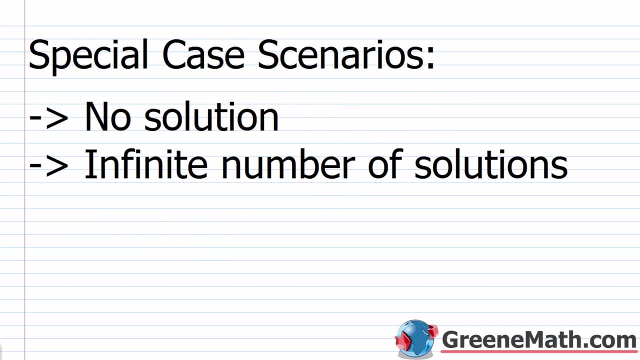 this does in fact equal 8. you get 8 equals 8, so this one checks out as well. so we can say that the ordered pair, 4 comma 2, is in fact the solution for this system. alright, so now that we looked at two basic problems. 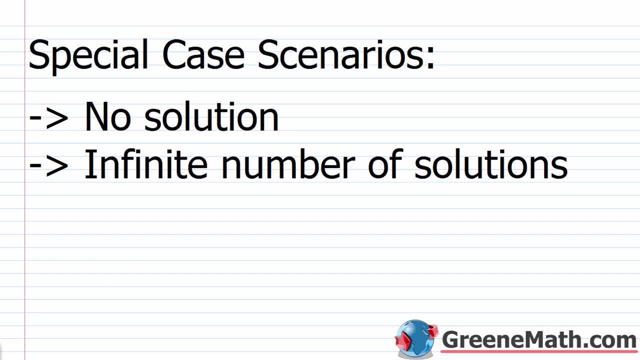 I want to kind of get into some special case scenarios. so one scenario you're going to come across is where you have no solution, and then another scenario you're going to come across is where you have an infinite number of solutions. so, when we think about the types of problems, 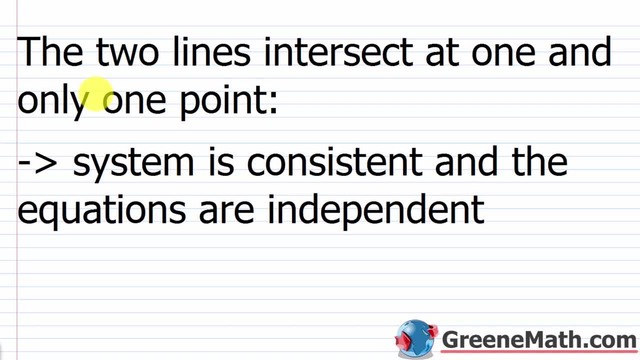 we're going to encounter. most of the time, or I would say the vast majority of the time, the two lines will intersect at only one point. so these are the two examples we just looked at. the system is consistent and the equations are independent. ok, so the system is consistent. 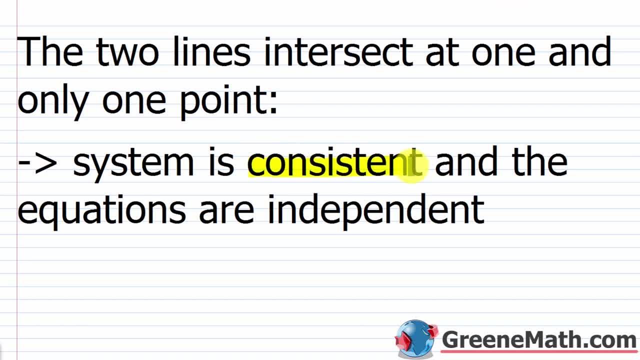 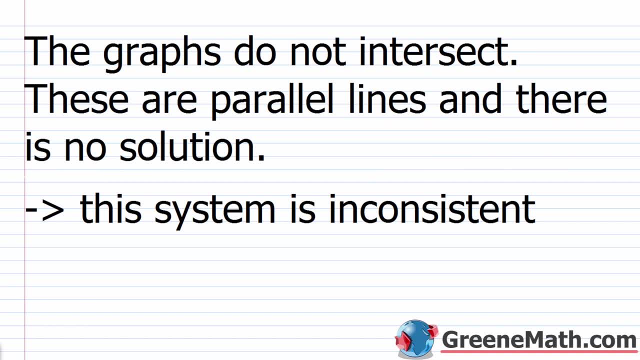 let me highlight that the system is consistent and the equations are independent. now, here's one of the special case scenarios, so you'll get this thrown at you all the time too. the graphs do not intersect. the reason for that is these are parallel lines. remember parallel lines, do not. 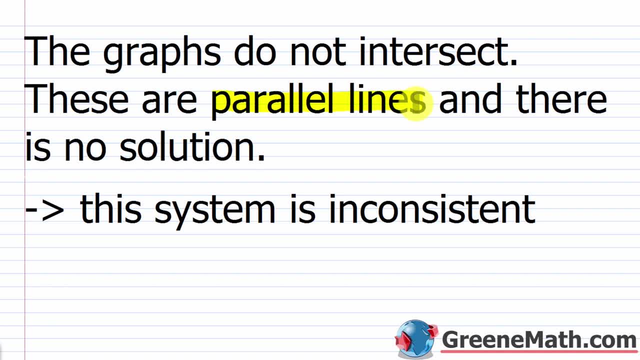 intersect by definition. so if they don't intersect, that means there's not going to be a point that is on both lines and therefore there is no solution for the system. so I have here: these are parallel lines and there is no solution. ok, now you'll say that this system is 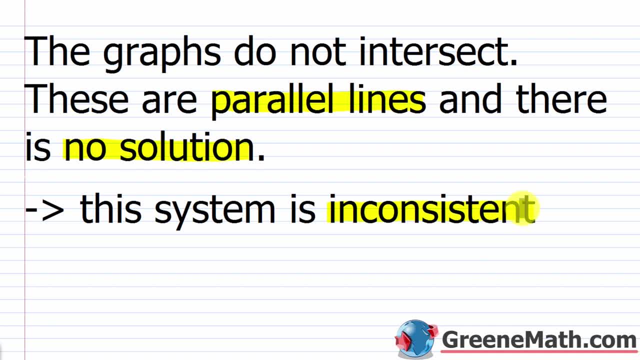 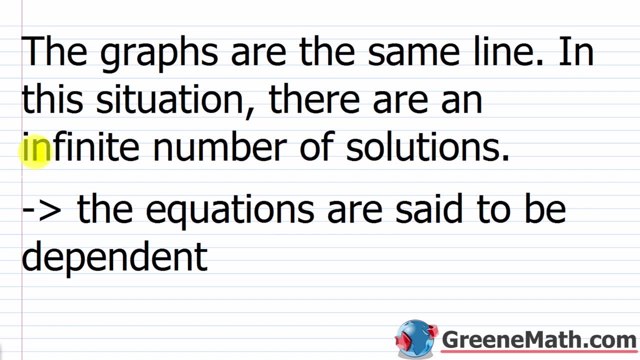 inconsistent. remember the last scenario? we had a system that was consistent. here there's no solution, so the system is inconsistent. so the final scenario you're going to deal with is that the graphs are the same line, so in this situation, there are an infinite number of solutions. 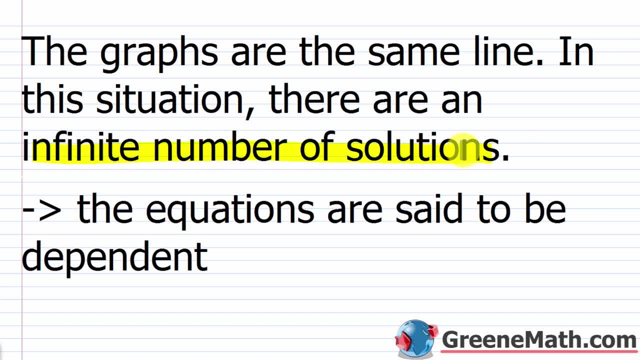 now you might say: what do you mean? they're the same line. it doesn't make any sense. what's going to happen is you're going to start out with two equations that look different, but really it's the same equation that they've algebraically manipulated to look different. and the way you 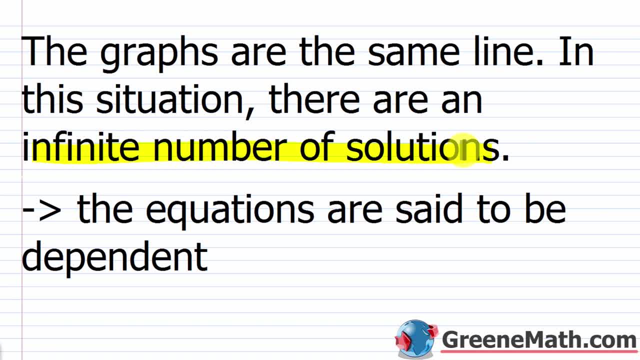 guard against this is you put everything in slope intercept form. that's going to tell you right away if you have one of these special case scenarios. so if you put everything in slope intercept form, not only are you going to guard against the special case scenarios, you're also going to be able to graph. 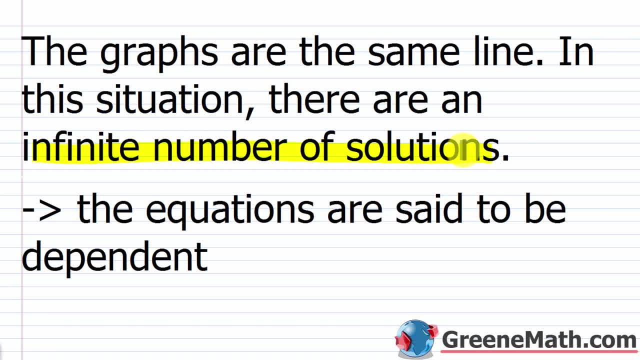 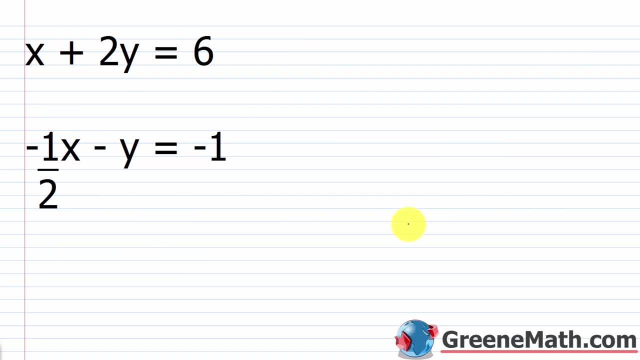 anything you're going to deal with very, very quickly, alright. so these equations are said to be dependent. ok, they're dependent, alright. so let's look at a special case scenario. so we have x plus 2y equals 6 and we have negative 1 half x minus y. 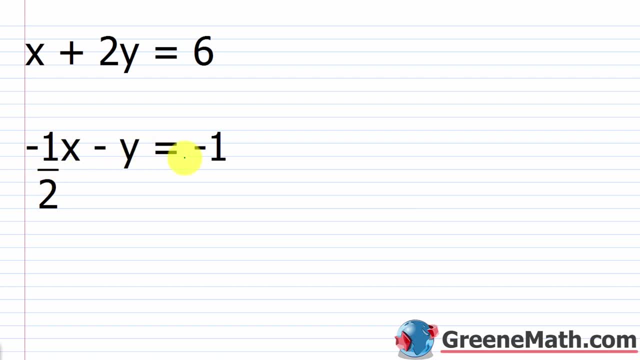 equals negative 1. so let's solve each one for y. so for this one I would say: x plus 2y equals 6. let's subtract x away from each side of the equation. this is going to cancel. I'll have: 2y is equal to. 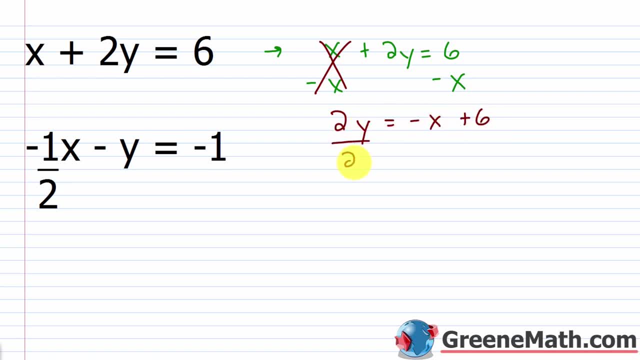 negative x plus 6. we want to divide both sides by 2. so what's going to happen is this is going to cancel. with this, I'll have y is equal to. we'll have negative 1. half x plus 6 over 2 is 3. 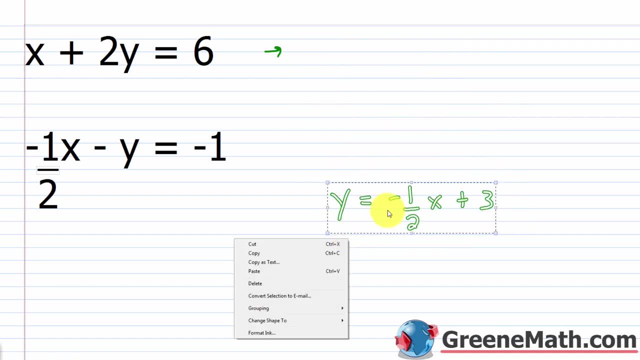 let's erase this real quick and let's drag this up here. so now let's solve this one for y as well. so we have negative 1 half x minus y equals negative 1. so let me add 1 half x to both sides of the equation. 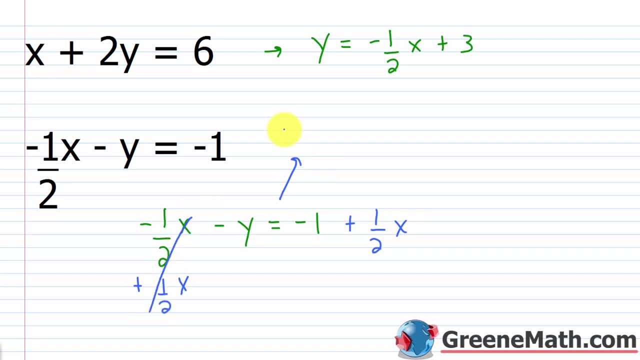 and I'll continue this up here. this will cancel. I'd have negative. y is equal to. you'd have 1 half x minus 1. now all I need to do is multiply both sides of the equation by negative 1 so I can get y by itself, or you could divide. 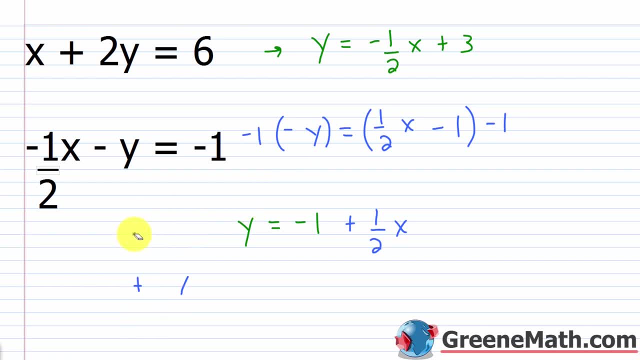 by negative 1. whatever you want to do, let's erase all this. so negative 1 times negative, y is y and this equals negative 1 times 1. half x is negative, 1 half x. and then negative 1 times negative: 1 is positive. 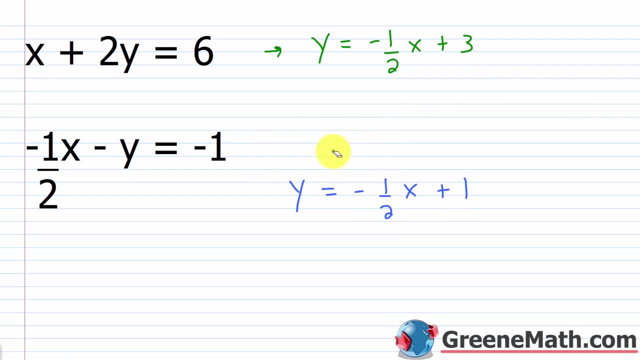 1. so I want to erase this and drag this up here and I want you to observe something: we did a lesson where we talked about parallel lines and hopefully you remember how you can determine if you have parallel lines. the two lines have the same slope but a different y intercept. 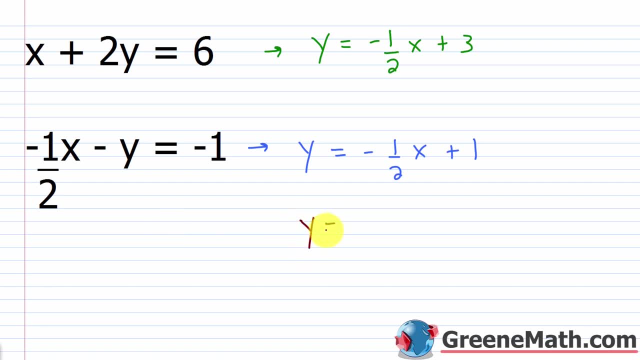 so if I look here again, if it's in the format of y equals m, the slope times x plus b, the y intercept. well, the slope is given as the coefficient of x in each case, and in each case here I have the same slope, negative, 1 half and negative. 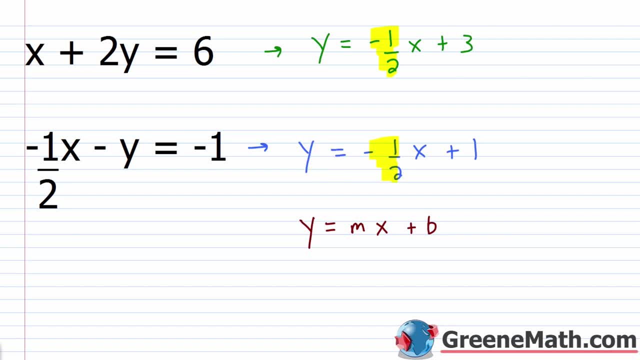 1 half. but the y intercepts are different. here the y intercept would occur at 0 comma 3, here it would occur at 0 comma 1. so same slope, different y intercept, parallel lines. so if you're on a test and you solve these for y and you see, 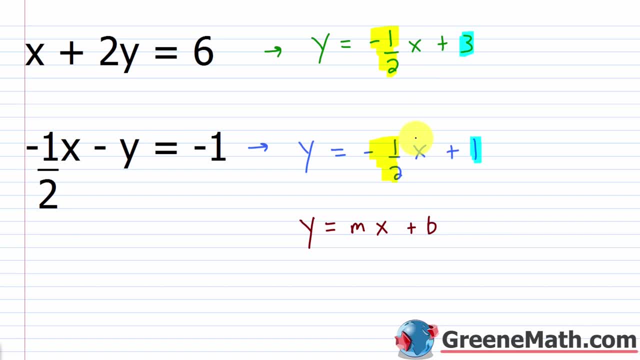 there's the same slope, different y intercepts, you can stop and you can put no solution. there's no solution. parallel lines will never intersect, so there's no ordered pair that's going to work in this one, that also works in this one. not going to happen. you can also put the. 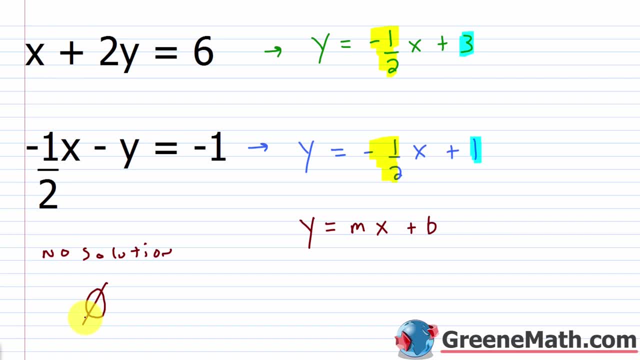 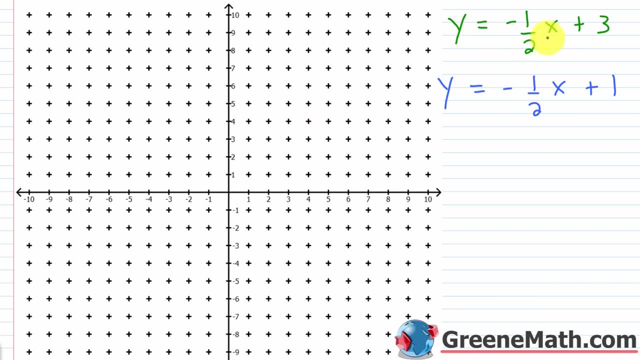 symbol for the null or empty set. now, for the sake of completeness, let's go ahead and graph these so we can see what they look like. for the first one we have: y equals negative, 1, half x plus 3, so the y intercept occurs at 0 comma 3. 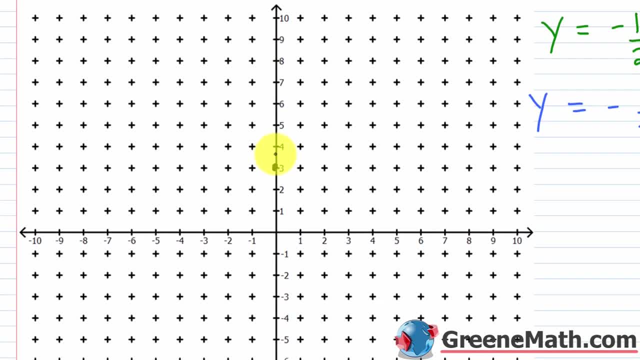 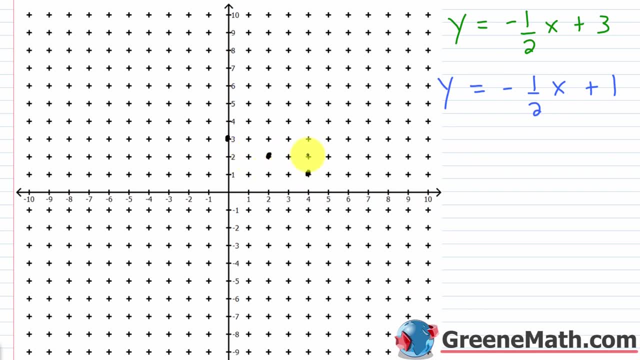 so that's right here. and the slope is negative 1 half. so down 1 to the right 2, down 1 to the right 2. or remember, negative over positive is the same as positive over negative. in the end it's just negative. so I could put the negative in the denominator. 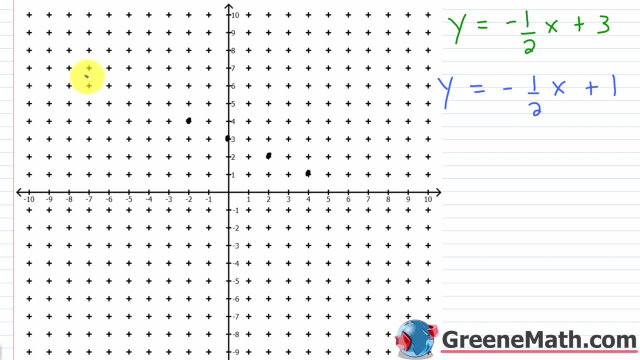 and I could say I could rise 1, go to the left 2. alright. so let me label this guy. this is: y equals negative 1 half x plus 3, alright. the next one was y equals negative 1 half x plus 1. so the y intercept for that one. 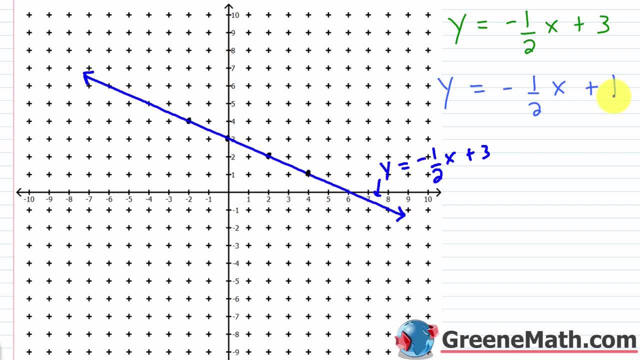 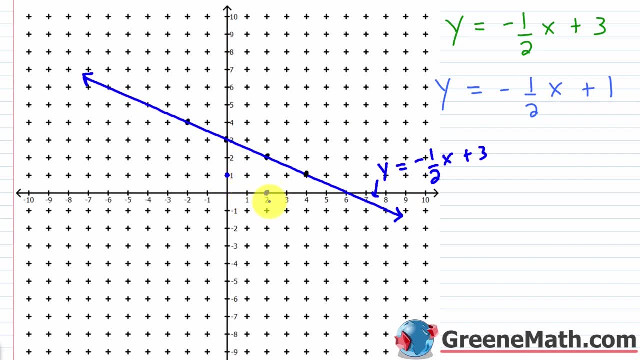 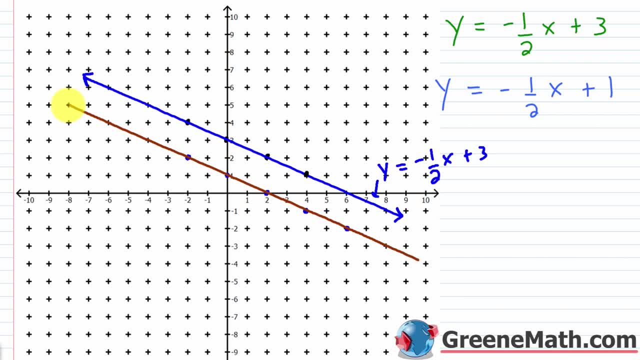 alright, so let me label this guy. so let me label this guy. so let me go ahead and label this one as well. this is: y equals negative 1, half x plus 1. you notice that you have parallel lines here. you can see it: these lines will never, ever ever intersect. 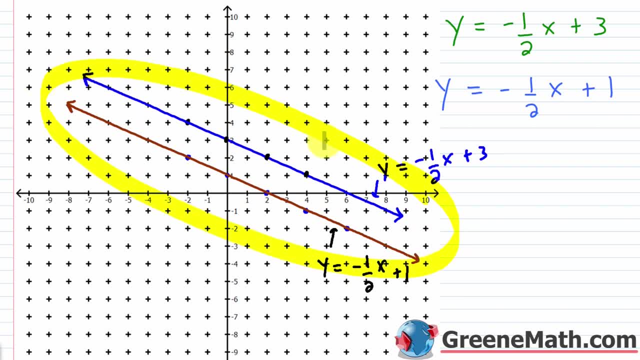 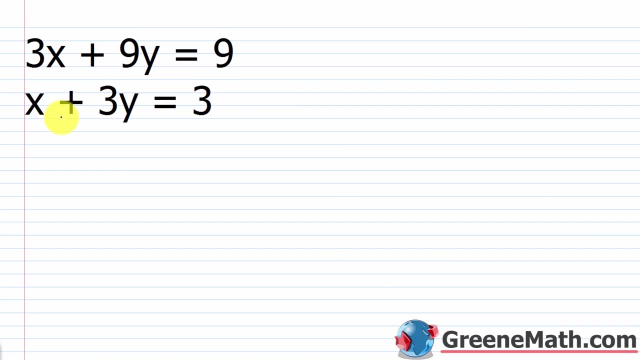 these lines will never, ever ever intercept. the space between them will always be the same. so we have parallel lines. so for this system there is no solution. alright, for the next one one, We have 3x plus 9y equals 9.. And we have x plus 3y equals 3.. So again, let me solve each one. 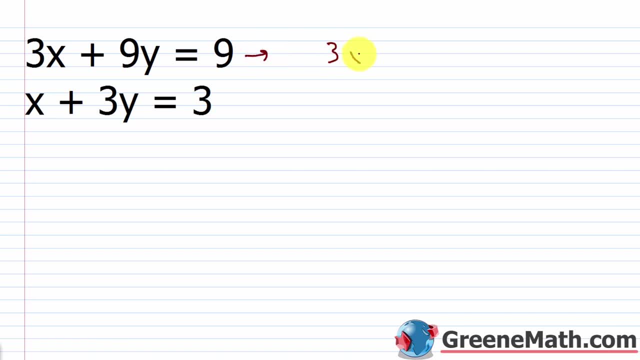 for y. So if I solve this for y, I would have 3x plus 9y equals 9.. Let me subtract 3x away from each side of the equation And this is going to cancel. We will have: 9y is equal to. we have 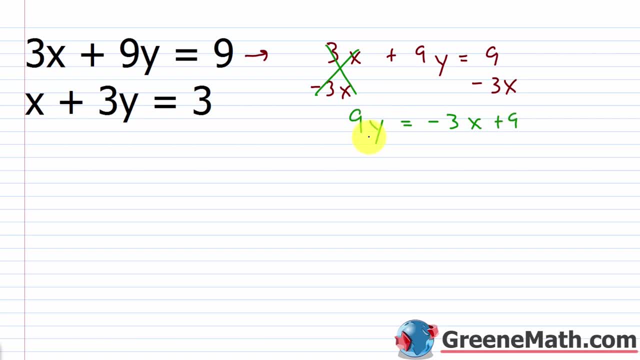 negative, 3x plus 9.. Let's go ahead and divide both sides of the equation by 9.. This is going to cancel. with this We'll have: y is equal to negative, 3 over 9 is negative 1. third. Then times x, 9 over 9 is 1.. So plus 1.. Let me erase all of this. All right, now let me solve. 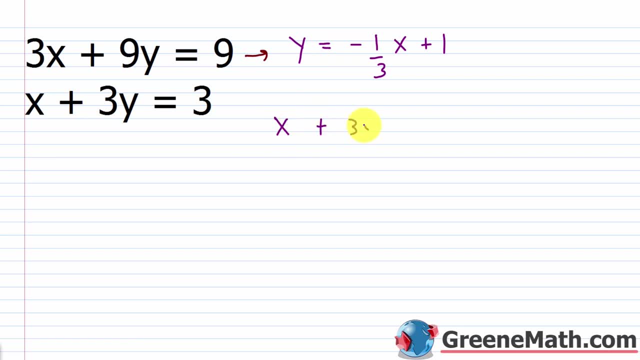 this one for y as well. So we have x plus 3y equals 3.. And so I will subtract x away from each side of the equation And then I'm going to divide both sides of the equation by 9.. That'll cancel. I'll have: 3y is equal to negative x plus 3.. Divide both sides of the equation by 3.. 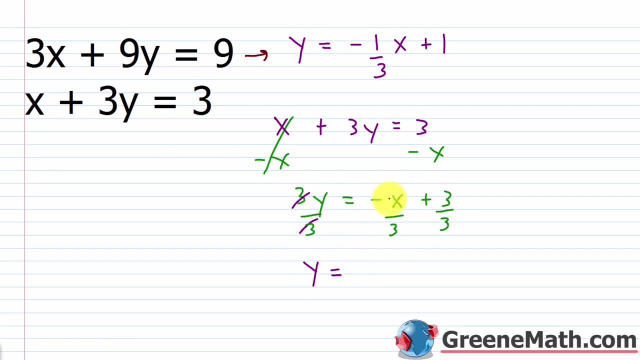 And this will cancel. with this, I'll have: y is equal to negative x over 3.. We can basically say this is negative 1. third x plus 3 over 3 is 1.. So let's erase all of this, Let's drag this up. 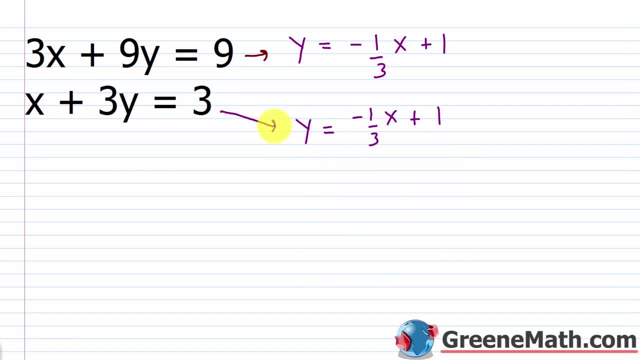 here. And what do we notice here? We have the exact same equation. So whatever ordered pair works here will work here, And there's an infinite number of solutions for a linear equation in two variables. So, because there's an infinite number of solutions for this, 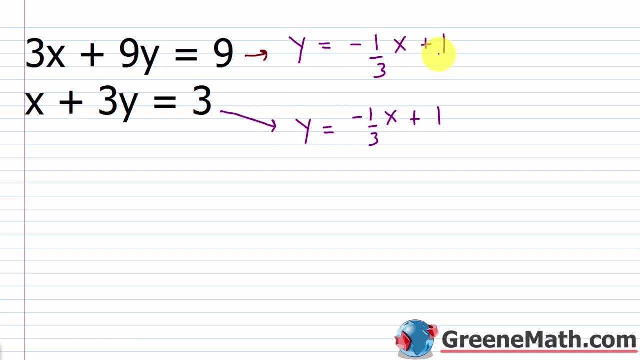 guy, and this guy is the same as this guy. there's an infinite number of solutions for the system, because the system just contains the same equation twice, So there's an infinite number of solutions here. So we will say there's an infinite number of solutions. 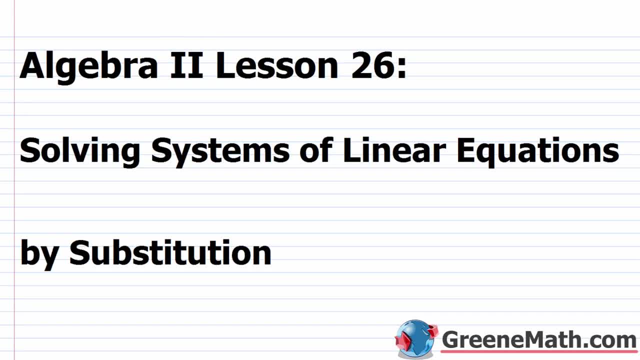 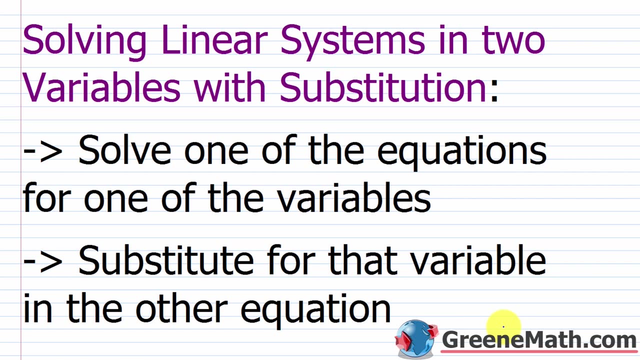 Hello and welcome to Algebra 2, Lesson 26.. In this video we're going to learn about solving systems of linear equations by substitution. So in our last lesson we reviewed how to solve a system of linear equations in two variables using the method known as graphing. Now, if you 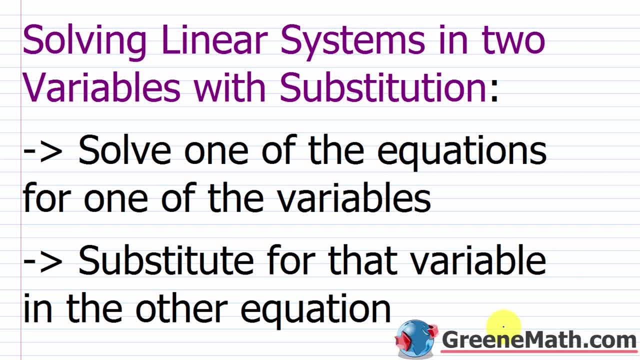 took an Algebra 1 course. that was nothing new for you. But if you took an Algebra 2 course, you took an Algebra 3 course And, of course, if you took Algebra 1, substitution is not new for you And it's also not going to be new when we cover elimination as well, But it's. 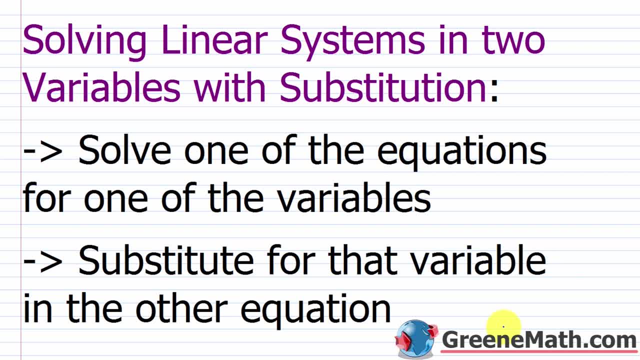 important to review these concepts. so when we start looking at tougher material, it's fresh in your mind. Now the one thing I'm going to say about graphing. you might say, well, why don't we just use graphing? We've already learned one method. Why not just use? 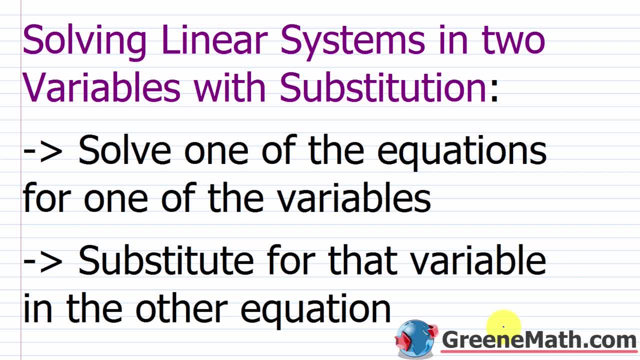 that. Forget about the rest. Graphing is very inefficient, If you can imagine having a piece of paper, a ruler and a pencil and trying to find a solution. that's, let's say, the ordered pair: 200, negative 400.. Okay, 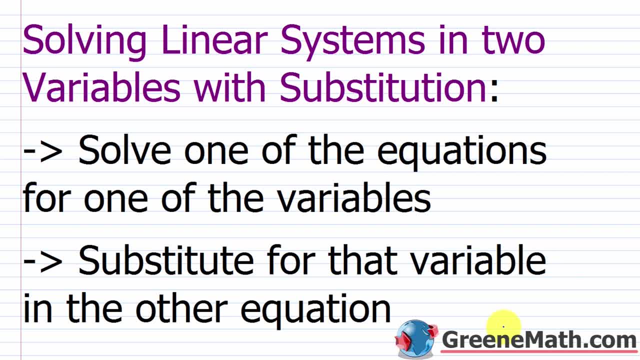 it's very hard to do that. It's not impossible but it's very difficult. Or let's say you had one half comma negative two fifths, something like that. It's very hard to use graphing unless you have a small, clean, integer answer. And those were the examples that I gave And I 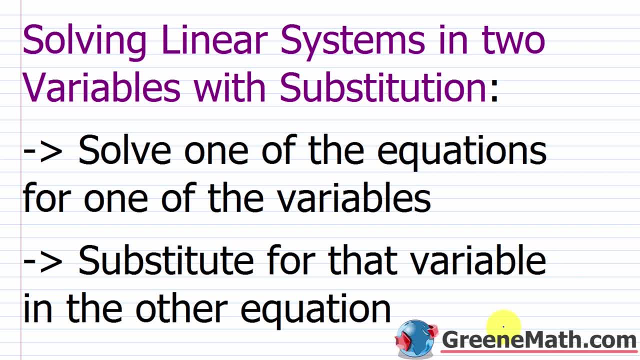 give them on purpose, so that you can just get a conceptual understanding. You don't want something tedious. You know, forget about it, I'm not going to do this. So we turn to substitution as an algebraic method. This is something you can use, no matter how big or small something is. fractions: 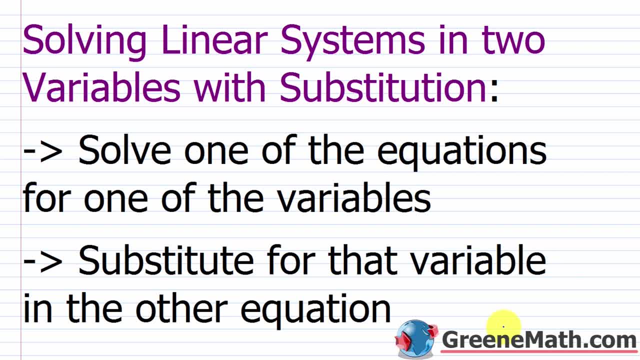 decimals, whatever you want. you can use substitution. Now I am going to say substitution works best when you have a coefficient for one of the variables, that's a one or a negative one. Okay Now, with that being said, let's kind of dig into this. So, solving linear systems in two. 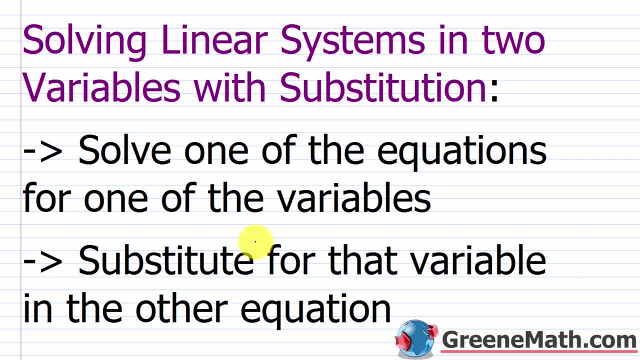 substitutions. So the first thing that we want to do, we want to solve one of the equations for one of the variables. So it doesn't matter which equation you use, It doesn't matter which variable you start out with. Okay, It is going to be helpful, as I just mentioned, if you have a 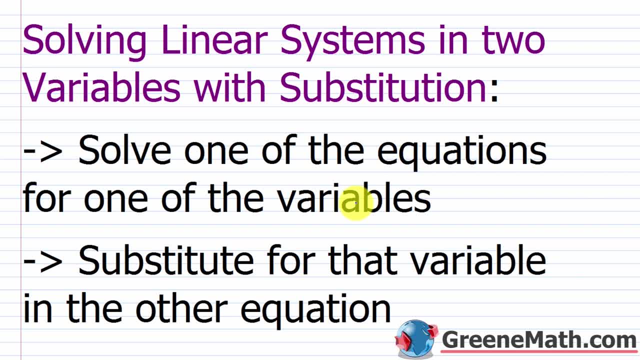 variable that has a coefficient, that is one or negative one. you want to use that because it's easy to solve for that variable, But otherwise you can use whatever you want. Now, after you've done that, you want to solve one of the equations for one of the variables, So you want to solve. 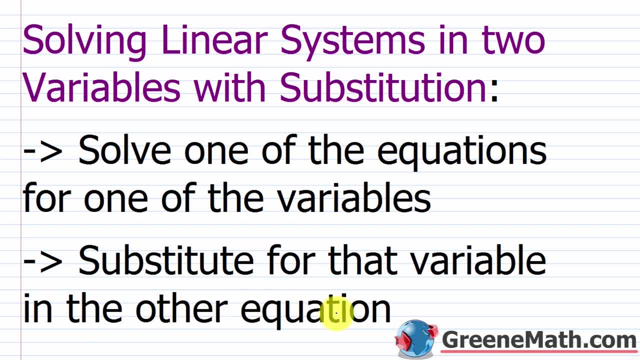 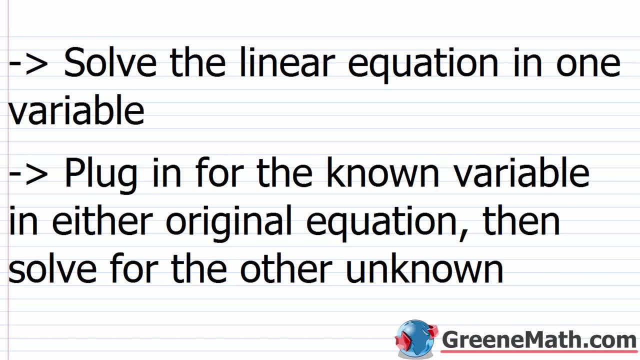 for that variable in the other equation. Now, once you've finished that step, you're going to notice that that equation you're working with is a linear equation in one variable, something we've been solving forever now. So we want to solve the linear equation in one variable. And then what? 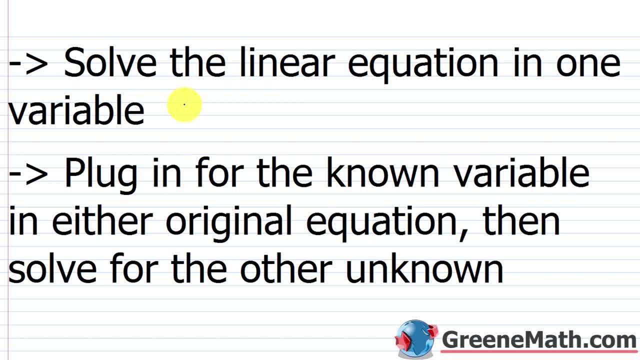 that is going to do is give us a solution for one of the variables. So once I have that, I plug in for the known variable in either original equation- It doesn't matter which one I use- Then solve for that. I figured out the ordered pair. that is a solution for this system. And again I say ordered. 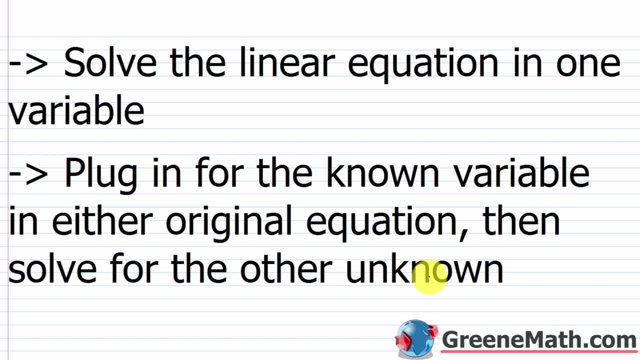 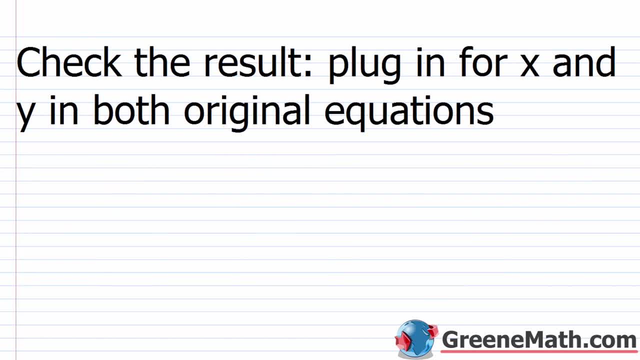 pair, because usually that's what you're going to get. You know, you have special case scenarios where you have no solution and an infinite number of solutions. I'm talking about the case where you have one solution, All right. So the last thing we want to do- and it's very important you do this- 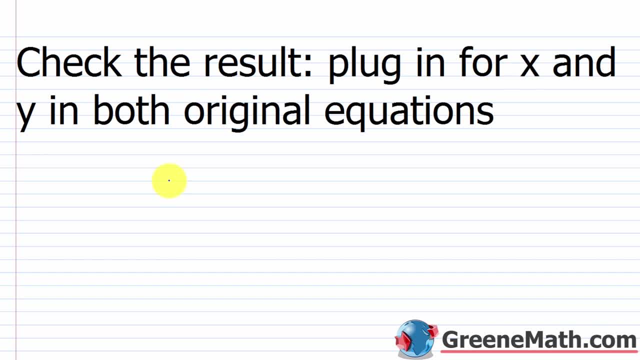 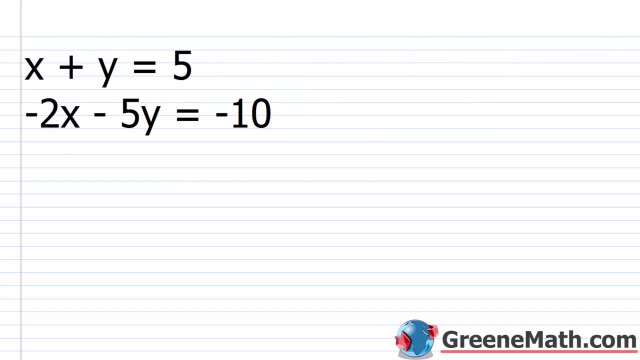 check the result. So you want to plug in for X and Y in both original equations. All right, So let's take a look at the first example. So we have our linear system here in two variables. So we have x plus y equals 5, and we have negative. 2x minus 5y equals negative. 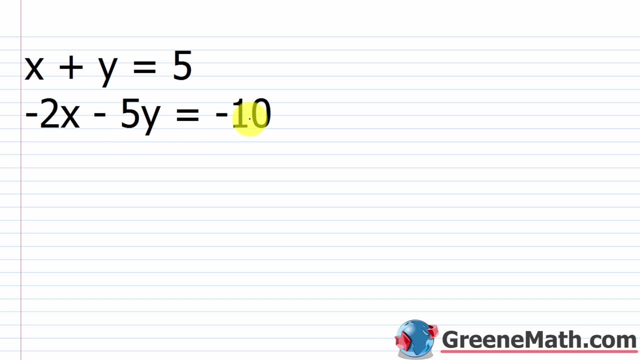 10.. So I would pick one of the equations and solve it for one of the variables. Now, if I look at this first equation- and I'm going to label this as equation 1, so I can refer to it- I'm going to 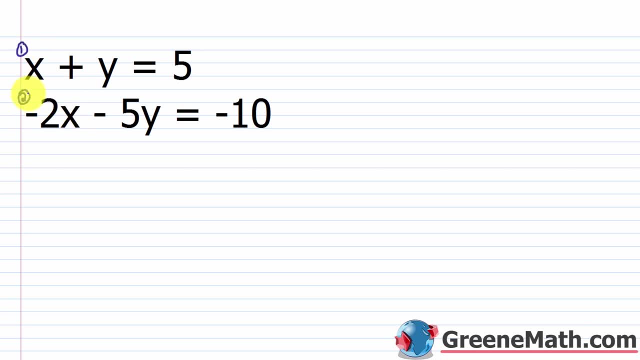 label this as equation 2, so I can refer to it. If I look at equation 1,, I notice that the coefficient for x and the coefficient for y is a 1. So it would make it pretty easy to solve for either one, So let's go ahead and just solve it for y. So if I have x plus y equals 5, and I solve that. 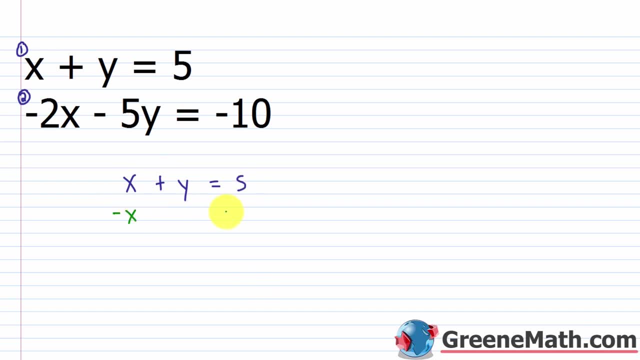 for y. we've been doing this for a while now. I just subtract x away from each side of the equation, and so this would become: y is equal to I'd have negative x plus 5.. Now I want you to think. 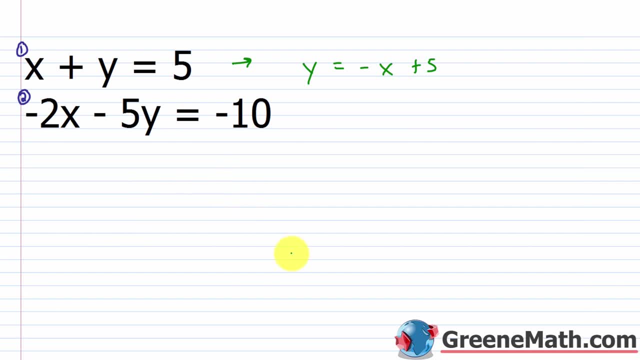 for a second. what the equals sign means- Equals is saying- is the same as: So y is the same as negative x plus 5.. It's like if I have money and I say a dollar is the same as four quarters. They are the same in value. They don't look the same, but they are the same. If I give a cashier 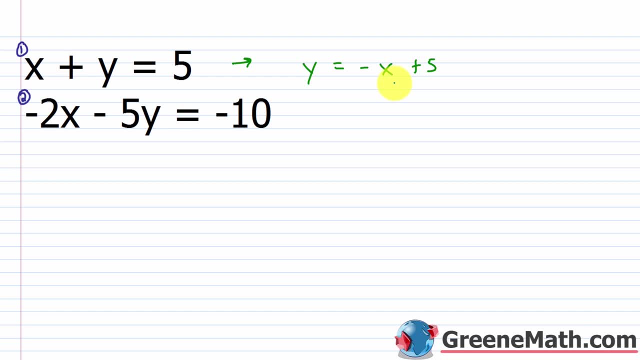 four quarters. if I give a cashier a dollar bill, I've presented the same value to the cashier, and so that is $1. Either way Okay. So now that we have solved this guy for y, I am going to plug into the other. 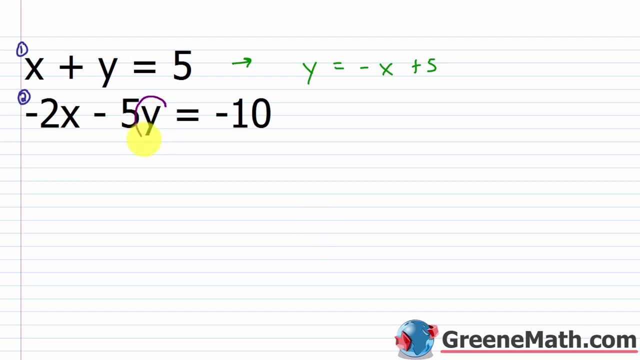 equation. Okay, So I'm going to plug in for y here Again, y equals this, So this is going to get plugged in there. That's all I'm doing. So I would have what An equation. 2, negative 2x. 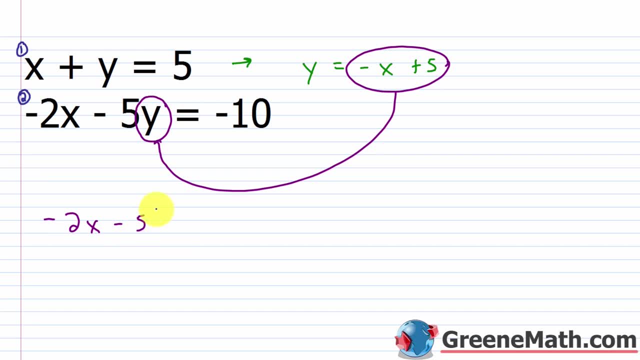 minus 5.. I've got to use parentheses here, because 5 is multiplied by y and y, is this Quantity negative x plus 5. And this equals negative 10.. So notice that I have substituted in for y in the second equation and the result here is a linear equation in one variable. 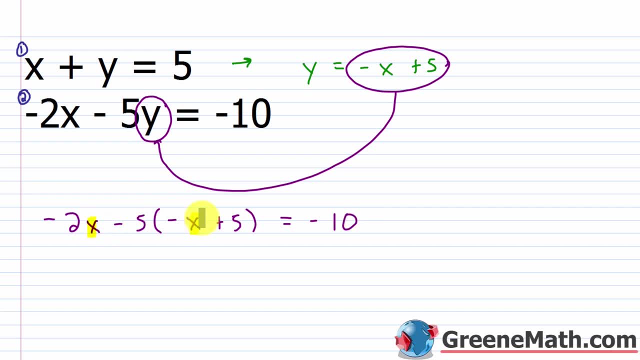 I now only have to deal with x, and that's pretty easy to do. So I have negative 2x. I have negative 5 times negative x, That's plus 5x, And then negative 5 times 5 is minus 25.. 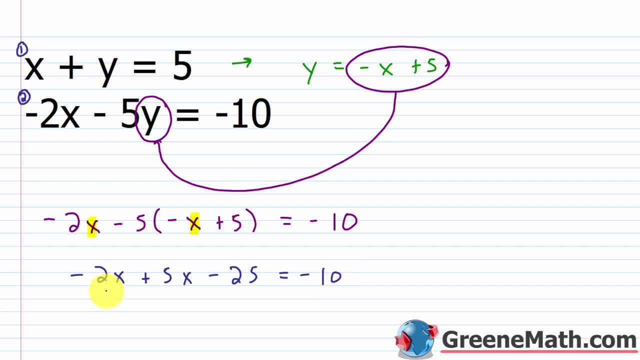 And this equals negative 10.. Combine like terms on the left: Negative 2x plus 5x is 3x And minus 25 equals negative 10.. Let's go ahead and add 25 to each side of the equation. 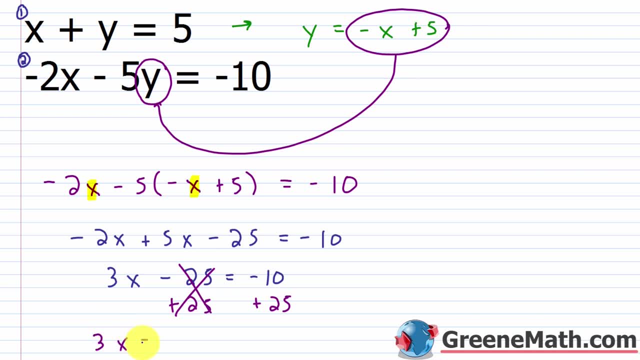 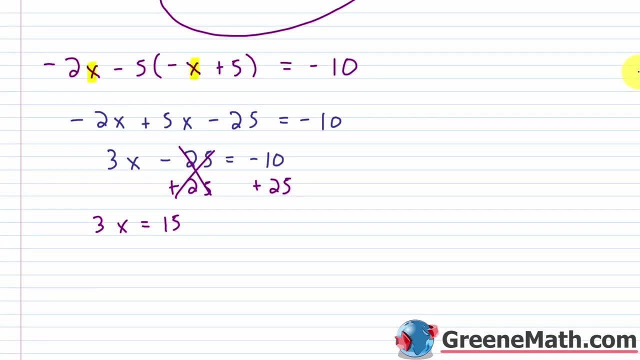 This will cancel. We'll have: 3x is equal to negative, 10 plus 25 is 15.. Let's go down and get a little room going. We divide both sides by 3, and we get x is equal to 5.. Now 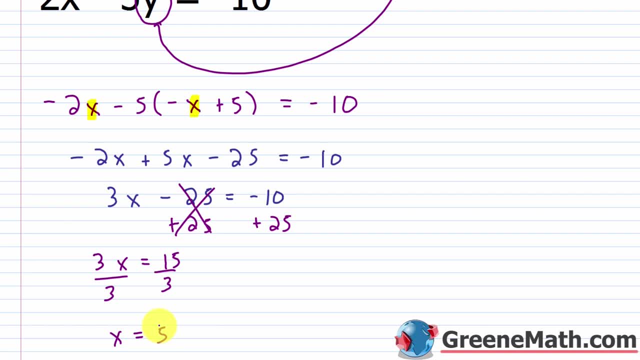 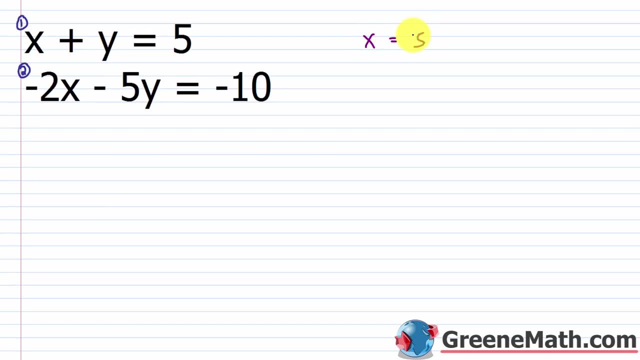 for the ordered pair. that is my solution to the system. I already know that x is 5.. Let me erase everything I've done to this point. So we know x is 5.. So as an ordered pair I'd have 5 comma something. Now how am I going to get this other something? 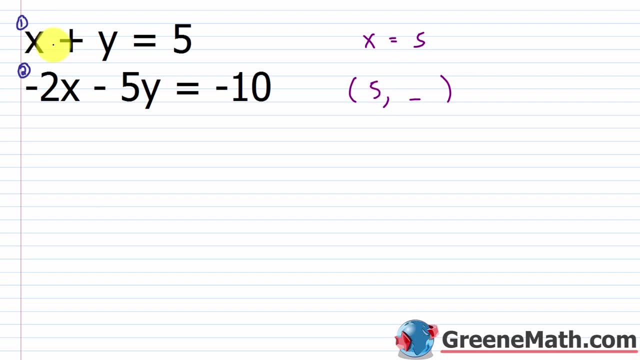 Well, 5 works as a solution for x in both equations if it's a solution for the system. So I can plug a 5 in for x here in equation 1 or here in equation 2 and solve for the unknown y. So let's go ahead and do it in equation 1, because it's a much simpler. 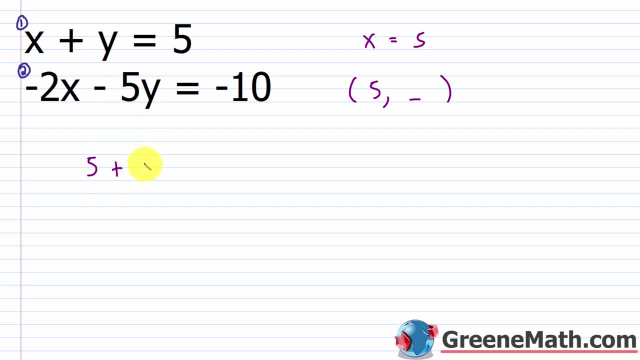 equation. So we would have 5 plus y equals 5.. Well, we know y equals 0, right, But we can go through the steps. Subtract 5 away from each side of the equation. This will cancel. You'll get y is equal to 5 minus 5 is 0. So 5 comma 0.. Now again, I want to check this to make sure that. 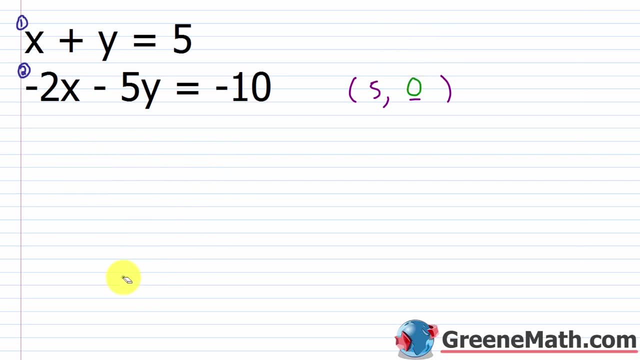 my answer is correct. So let's erase everything. We have x plus y equals 5. So x is 5 plus y is 0 equals 5. We know that's true, 5 equals 5. We just did that. So the other one you would have negative 2. So negative. 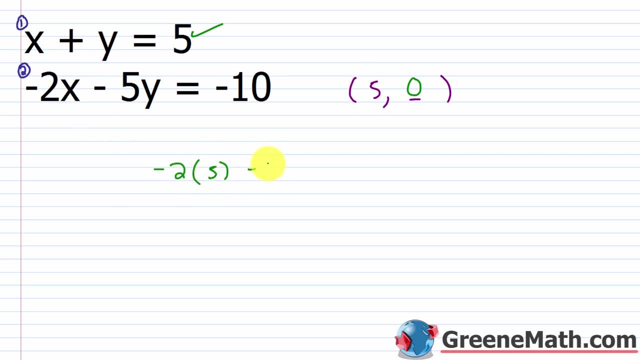 2 times plug in a 5 for x minus 5 times plug in a 0 for y equals negative 10.. Negative 2 times 5 is negative 10.. Of course, negative 5 times 0 is 0.. 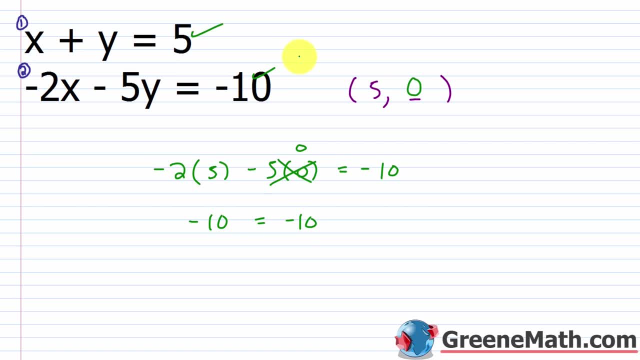 So I get: negative 10 equals negative 10.. So that's true as well. So we've verified that the ordered pair 5 comma 0 is the solution for this system. What if I would have- let me just throw this out here- What if I would have chosen equation 2 to start out with? And let's say, instead of solving, 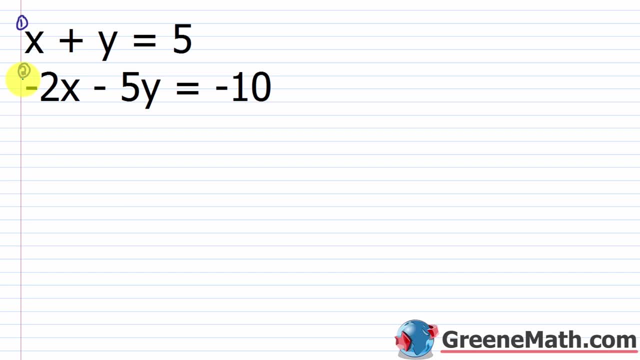 for y, I solved for x. Would I get the same answer? The answer to that is yes, Let's go ahead and do that. So I have negative 2x minus 5y. So I'm going to solve for x. So I'm going to add 5y to both sides of the equation. So this will: 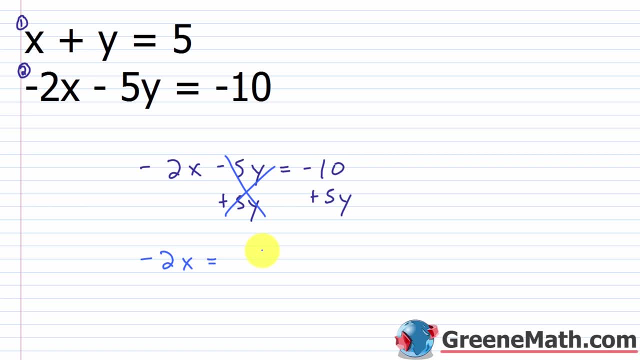 cancel. I'll have negative. 2x is equal to. you'll have 5y minus 10.. And then let's go ahead and divide both sides of the equation by negative 2.. So this is going to cancel. I'll have x is equal. 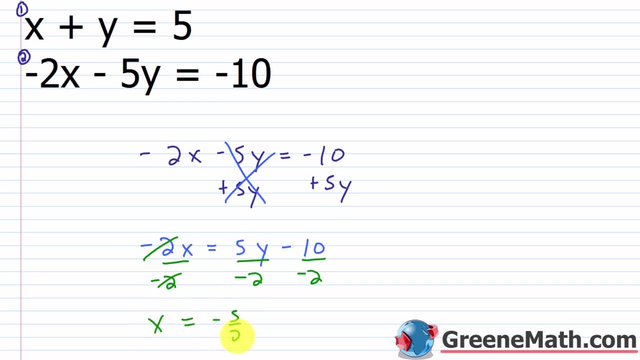 to 5 over negative 2.. Might as well just put negative 5 halves times y. Negative 10 over negative 2 is plus 5.. So this came from equation 2.. So I want to plug into equation 1.. And what do I want to plug in? 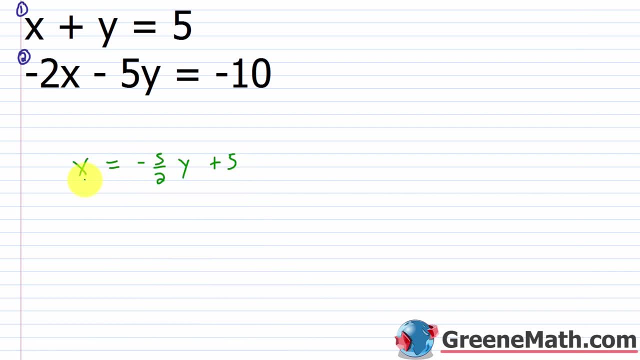 for I know that x equals x equals this value here. Negative 5 halves y plus 5.. So x is the same as that. So I'm going to plug in for x in this equation now And I'm going to plug this in. 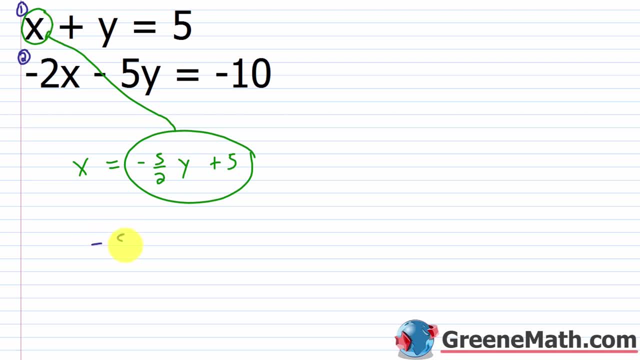 So when I do that, what happens? I have negative 5 halves y plus 5.. Then plus y equals 5.. So now I have a linear equation in one variable I just have a variable y, And again that's very easy to solve for So if I subtract 5 away from each side of the equation, 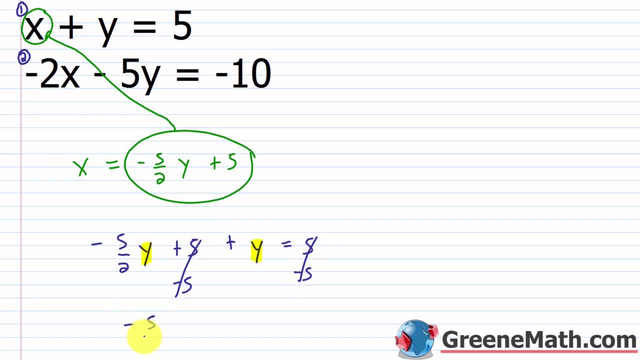 this will cancel, and this will cancel. You'll have negative 5 halves y plus y equals 0.. Now, before I do anything else, you know that the answer for y was 0. And you can see that the answer for y would be 0. So I'm going to plug in for x And I'm going to plug this in And I'm going to. 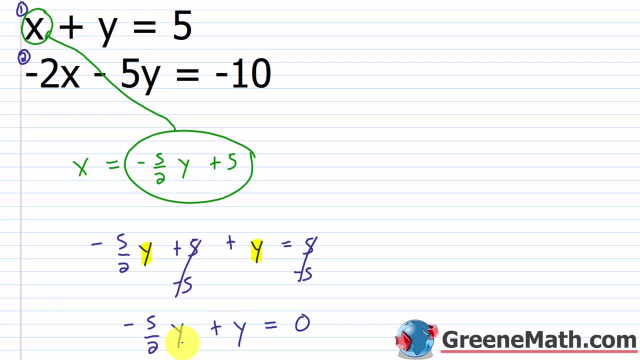 plug 0 here. No matter what, when I combine like terms, I'm going to have something: times y equals 0. that can only be true if y is 0.. OK, So you don't need to go any further. You've proved it. 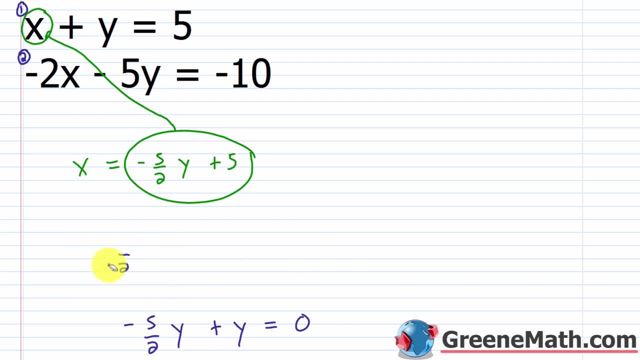 to yourself. But for the sake of completeness I'm going to go all the way here. So let me bring this up And let's go ahead and just multiply both sides of the equation by 2.. That'll be the easiest way to do this. So 2 times negative 5 halves is negative 5 and times y. 2 times y is: 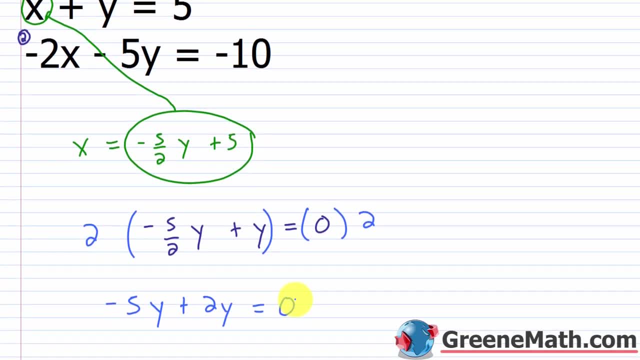 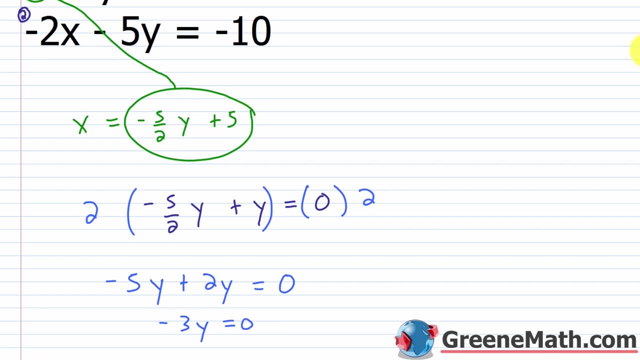 plus 2y, And this equals 0 times 2,, which is 0.. So negative 5y plus 2y is negative 3y And this equals 0.. And of course, to get y by itself, I divide both sides by negative 3.. This cancels. 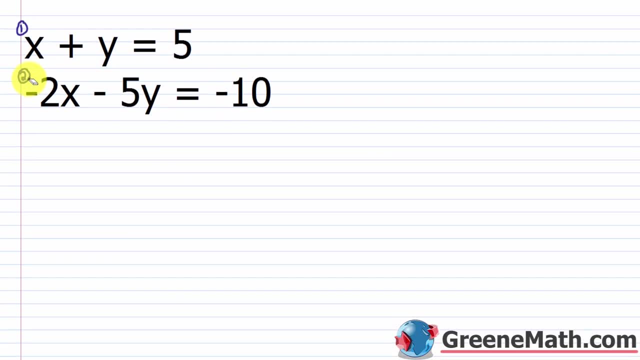 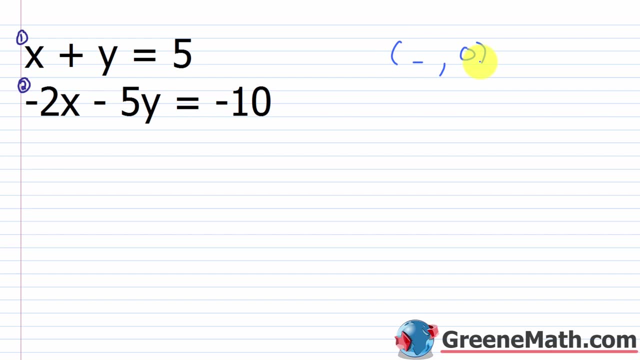 You get: y is equal to 0.. All right, So let's erase everything. And of course, we know that y equals 0.. So what is x? Again, plug in for y in either original equation- I can plug into this one- or 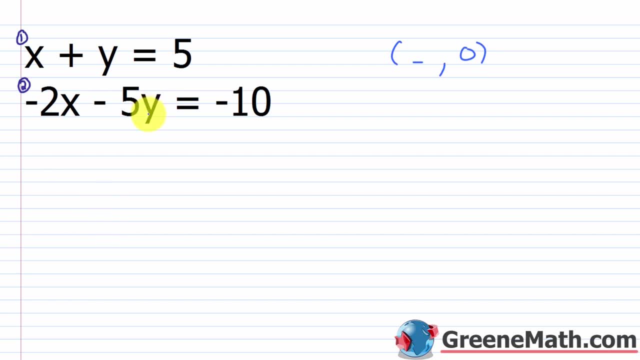 this one Doesn't matter, Let's go ahead and plug in for y in either original equation. Use the second one. So negative 2x minus 5 times 0 equals negative 10. So this will go away. I'll just have: negative 2x is equal to negative 10. Divide both sides by negative 2.. So this will: 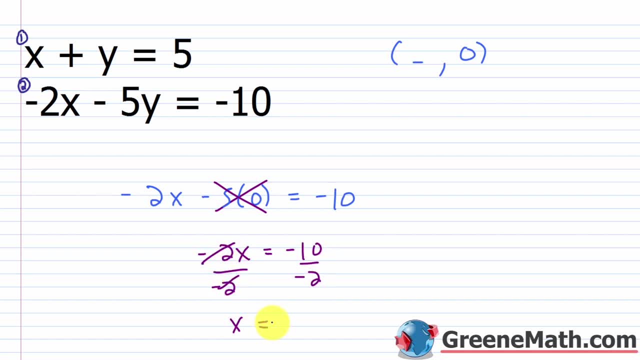 cancel: Negative 10 over negative 2 is 5.. So you'll have: x is equal to 5.. So I get 5 comma 0 as the ordered pair, as we already found. So any way you do it, you can solve for any variable. 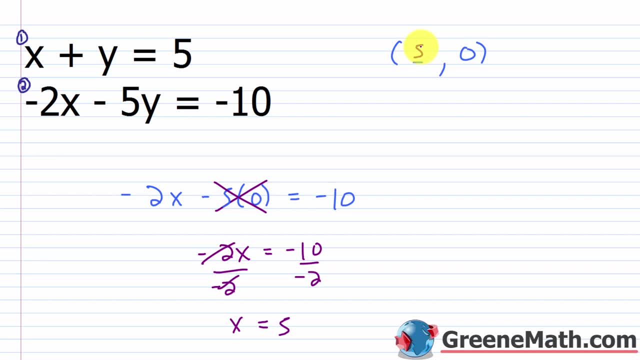 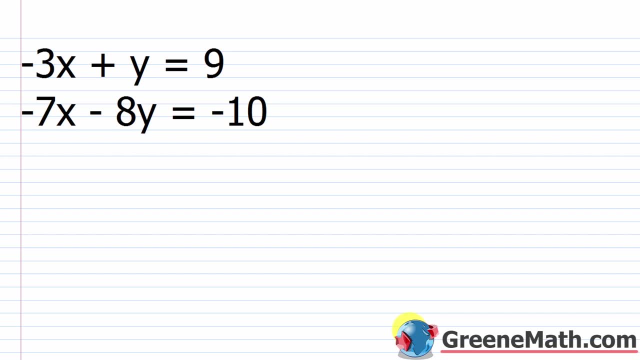 you want to start And you're going to plug in for that variable in the other equation. All right, For the next one. we have negative 3x plus y equals 9.. And we have negative 7x minus 8y equals. 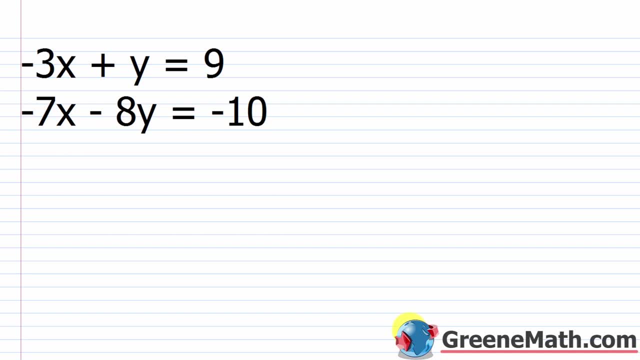 negative 10.. So the first thing I want you to notice here is that you have a coefficient of 1 on your variable y in. what I would like to say is the first equation, So I'm going to label this as equation 1.. This is equation 2.. Just for reference sake, I say: hey, equation 1, I'm talking about. 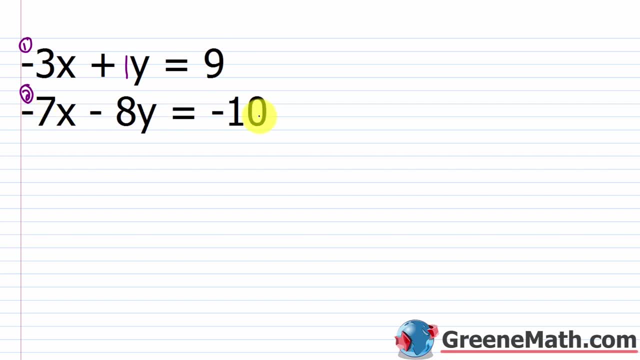 this one. Equation 2, I'm talking about this one, So I'm going to say hey. equation 1, I'm talking about this one. So the easiest thing to do here, since I have a coefficient of 1 there. 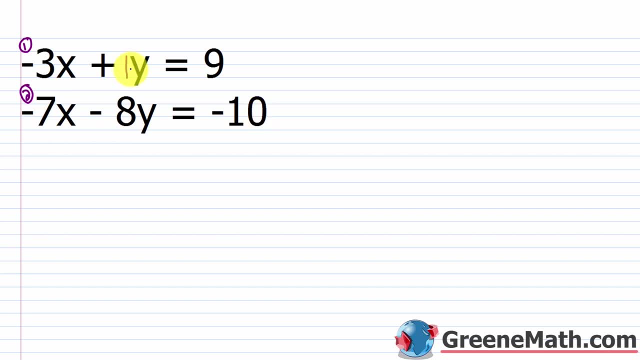 is to solve equation 1 for y, So let's go ahead and do that. Let's say that we have negative 3x plus y equals 9. All I've got to do is add 3x to both sides of the equation. 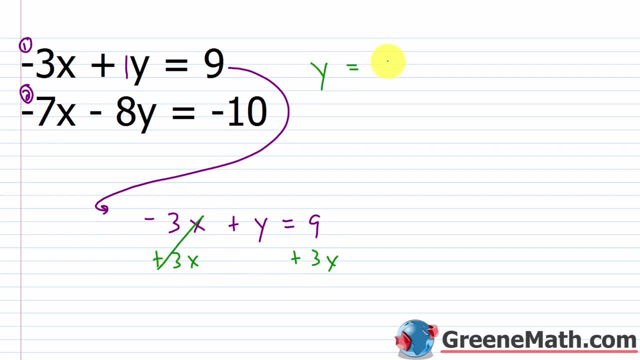 And this will cancel, I'll have: y is equal to 3x plus 9.. So that's super simple. All right, Now that I know what y is equal to, I'm going to add 3x to both sides of the equation. 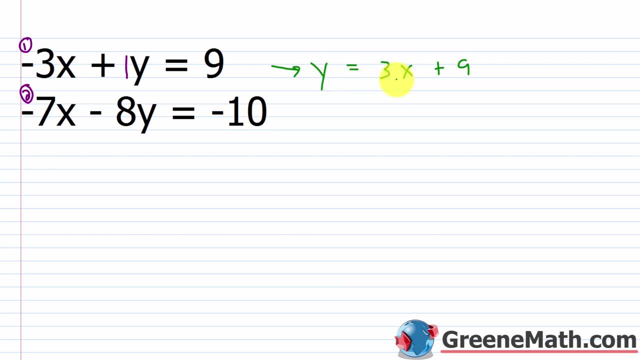 What y is equal to or what y is the same as. I can plug in for y in the other equation. So I'm going to plug this again: what y is equal to or what y is the same as in for this. So I would. 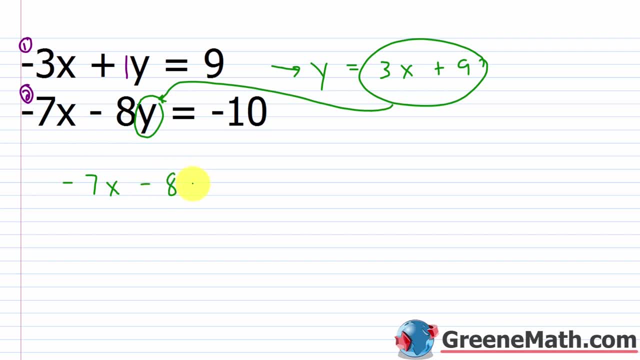 have negative 7x minus 8 times again, it's this whole quantity that y is equal to. So 8 is multiplied by that quantity. So I'm going to use parentheses: 8 times the quantity 3x plus 9.. 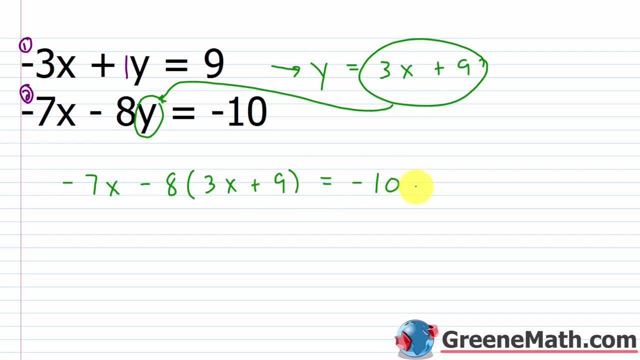 And this equals negative 7x. So let's go ahead and solve this equation: for x, You'll have negative 7x, And then you'll have negative 8 times 3x. That's negative 24x. Negative 8 times 9 is minus 72.. And this equals negative. 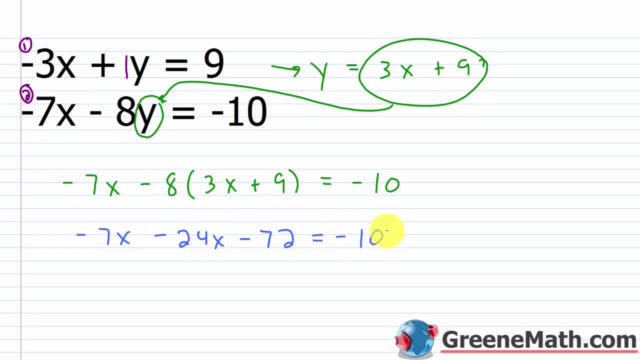 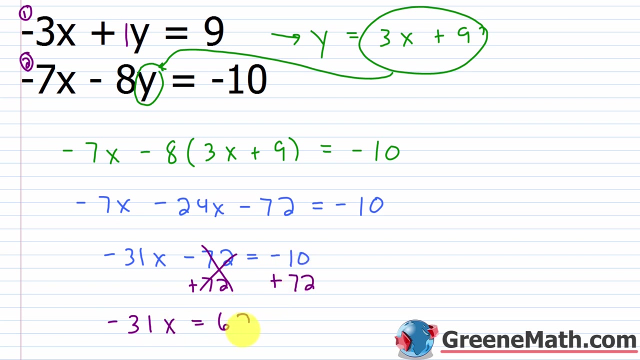 10.. So negative 7x minus 24x is negative 31x. So you'll have negative 31x minus 72 equals negative 10.. So let's go ahead and add 72 to each side of the equation. That'll cancel. You'll have negative 31x is equal to negative 10 plus 72 is 62.. So as a last step to 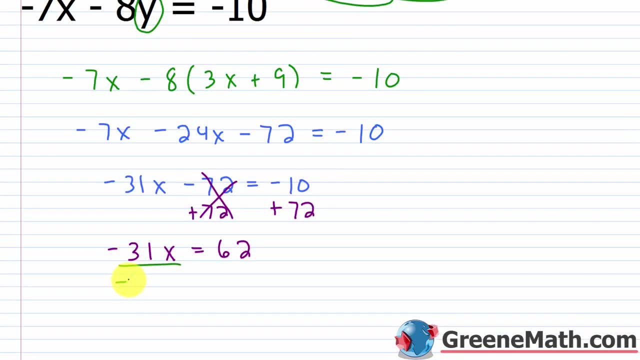 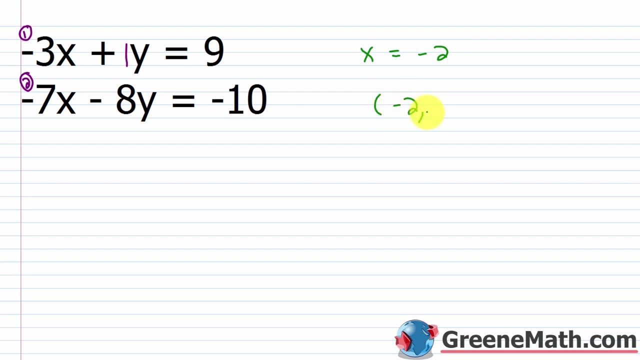 get x by itself. let's divide both sides by negative 31.. This will cancel And we'll see that x is equal to negative 2.. So let's go ahead and erase everything. So we already know that x is equal to negative 2, whereas an ordered pair would be negative 2. comma and then something. 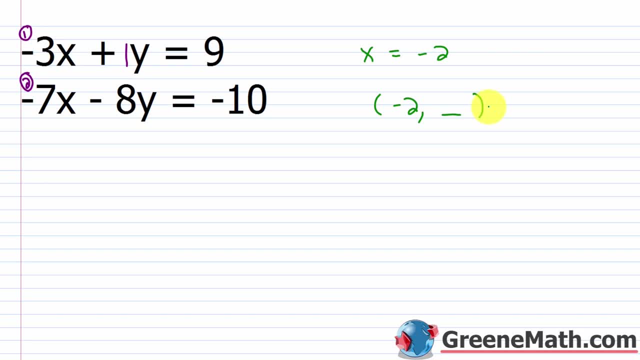 So I can plug in negative 2 in for x in either original equation. It doesn't matter, because in terms of the system I know x is equal to negative 2. So this one's easier to do in equation 1. Let's just use that. So you would have negative 3 times negative 2 plus. 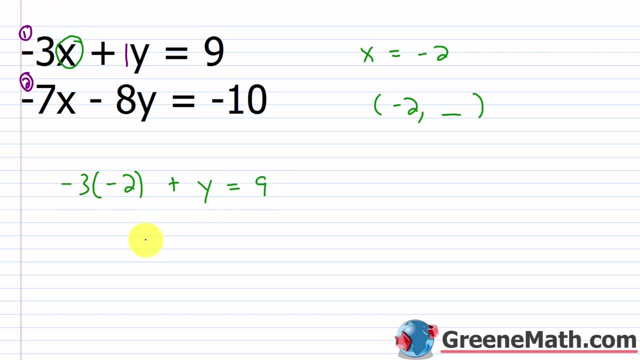 y is equal to 9.. So negative 3 times negative, 2 is 6, so you would have 6 plus y equals 9.. Subtract 6 away from each side of the equation and this'll cancel. We'll have y equal to negative. 2 into x minus zero times negative. 2 plus x is equal to 2.. You can change the answer if y equals zero, So you'll have 6 times negative 12.. You mean that 1 plus 2 is equal to y shall. 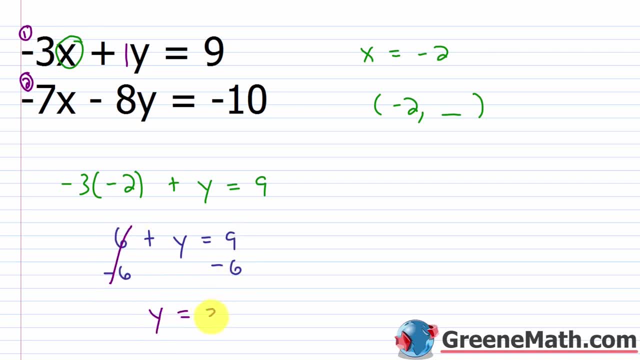 also replace those with x plus 1?? change the answer. Subtract 6 away from each side of the equation We'll have. y is equal to 9 minus 6 is 3.. So my ordered pair is negative 2 comma 3.. 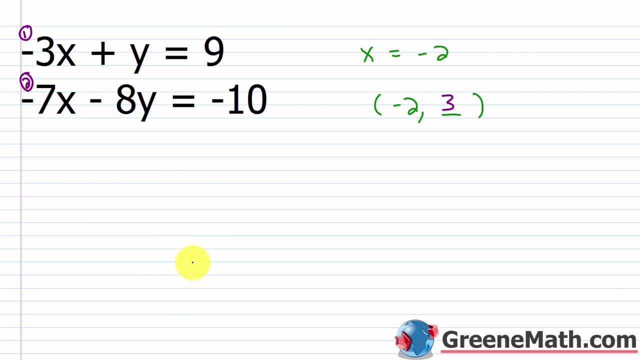 Let's erase all this. And so now we just want to check. We want to check an x value of negative 2 and a y value of 3 in each original equation. So I'm going to start with equation 1.. I'd have negative 3 times x. 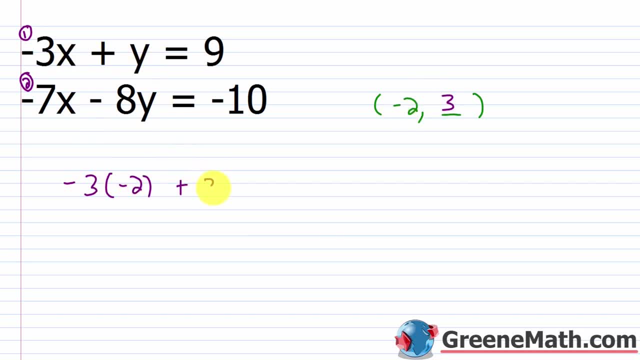 x is negative 2.. Plus for y, I have 3. And this should equal 9.. We know this works because we just did it. Negative 3 times negative 2 is 6.. 6 plus 3 is 9.. 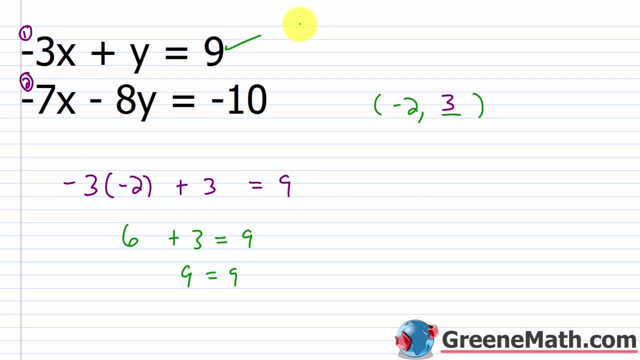 So you get 9 equals 9.. So this works out there All right. for equation 2, we have negative 7 times x. Again x is negative 2.. Then minus 8 times y, which is 3.. 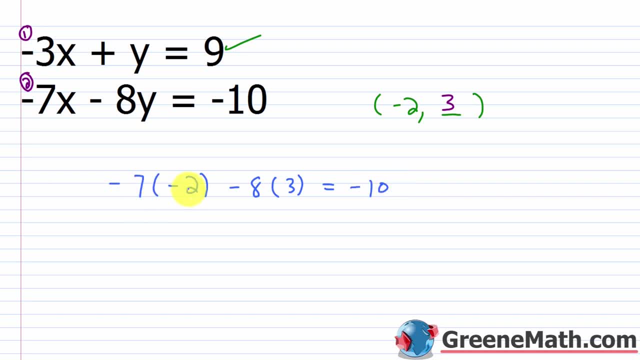 And this should equal negative 10.. Negative 7 times negative 2 is 14.. Negative 8 times 3 is negative 24.. And again, this should equal negative 10.. And it does right: 14 minus 24 is negative 10.. 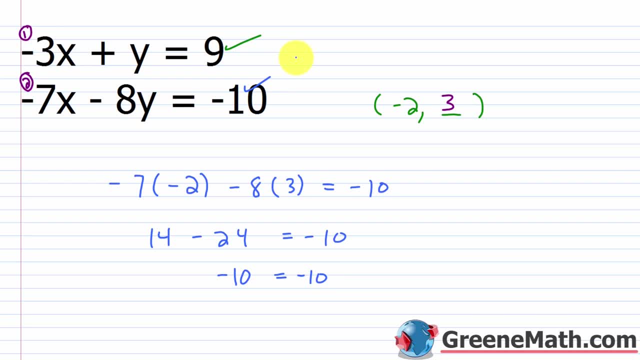 So you get negative 10.. So you can check this one off as well. So the ordered pair negative 2 comma 3, or an x value of negative 2 or a y value of 3, is the verified solution for this system. 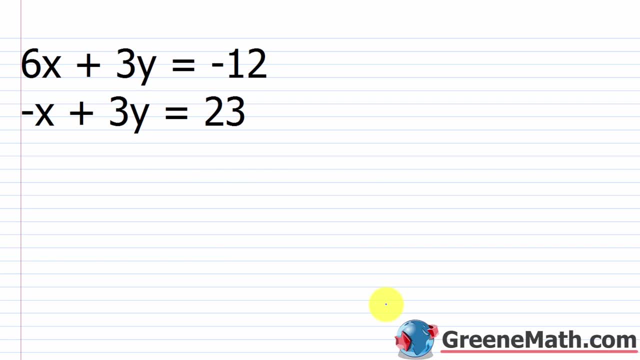 All right, let's take a look at another one. So we have 6x plus 3y equals negative 12. We have negative x plus 3y equals 23.. So again, if I find a variable in my system that has a coefficient of 1 or negative 1,, 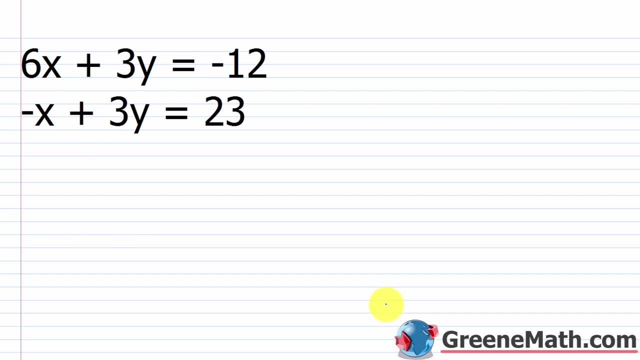 I want to use that as what I solve for. So here again, with negative 1 being there, I'm going to start out by looking at that. So, again, I'm going to label this as equation 1.. This is equation 2.. 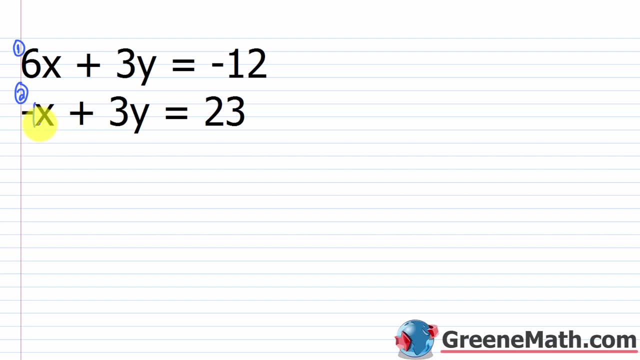 So with equation 2, I'm going to solve it for x. So I have negative x plus 3y equals 23.. And a couple of things I can do here. I can swap sides with this one and this one, Or I can just move 3y over and multiply both sides by negative 1.. 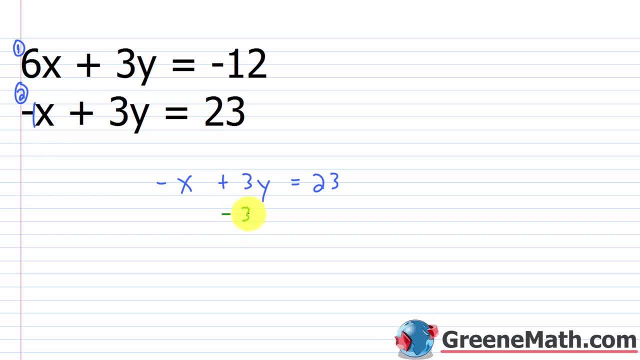 Whatever. Whatever you want to do, It doesn't matter. So let me just subtract 3y away from each side of the equation. That's how I'd like to do it. I'll have: negative x is equal to negative 3y plus 23.. 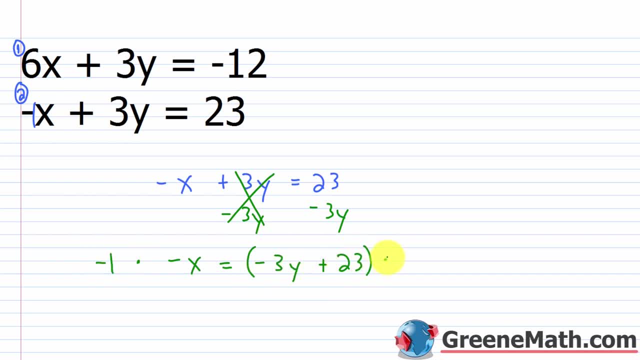 And let me just multiply both sides by negative 1.. So negative 1 times negative, x is of course x, And this equals negative 1 times negative. 3y is 3y. Negative 1 times 23 is minus 23.. 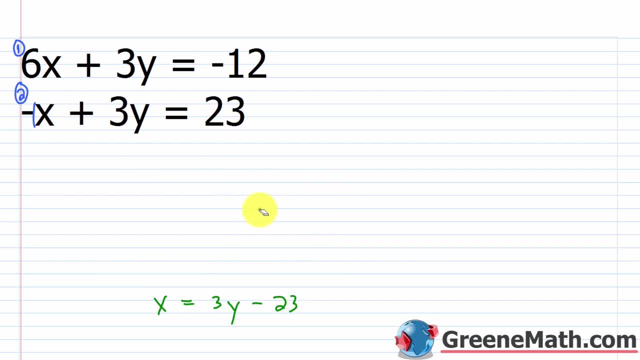 So I've solved this guy for x. So let me, I'm going to erase this, I'm going to drag this up, And if I've solved this for x, I can plug in for x in equation 1.. So I would have 6 times the quantity 3y minus 23.. 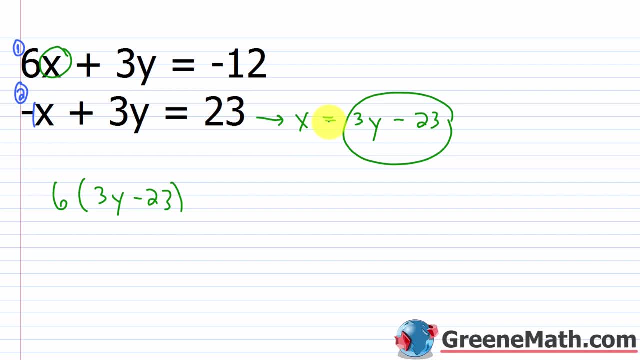 Again, x is equal to, or x is the same as, 3y minus 23.. So I can plug in for x there. So once I've done that, then plus 3y, I have a linear equation in one variable now. 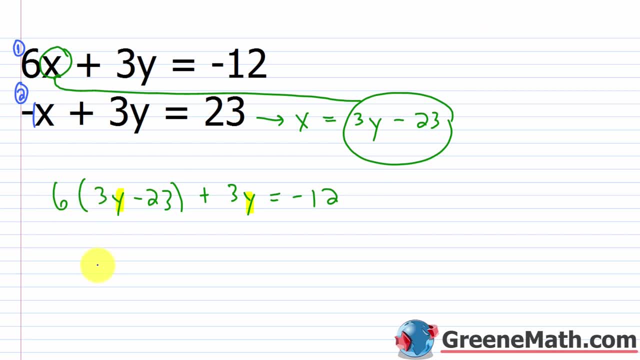 And it's easy to solve for that variable. So 6 times 3y is 18y, And then 6 times negative 23 is negative 138.. And then plus 3y equals negative 12.. So 18y plus 3y is 21y. 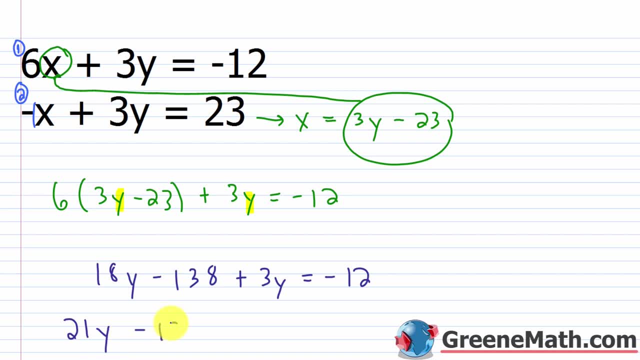 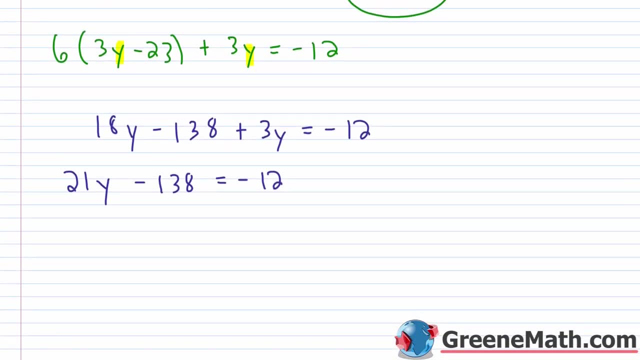 So I'll have: 21y minus 138 is equal to negative 12.. Let's scroll down Just a little bit. So now, if I add 138 to each side of the equation, this will cancel And I'll have: 21y is equal to negative. 12 plus 138 is going to be 126.. 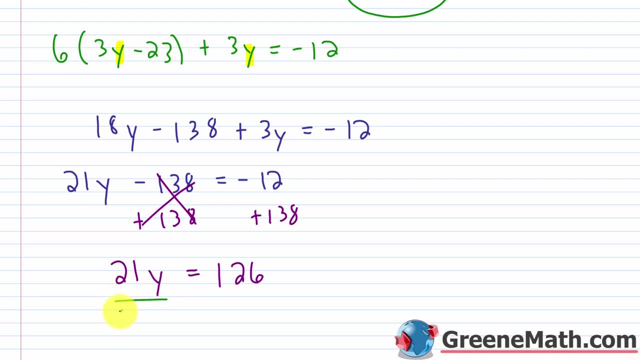 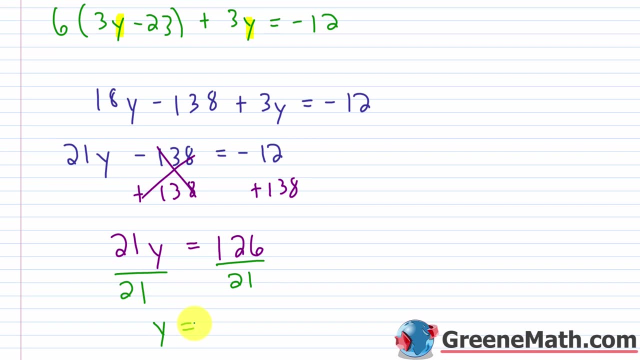 So as a final step to get y by itself, let's divide both sides of the equation by 21.. And we'll have that y is equal to 6.. Right, 126 divided by 21 is 6.. So y, y equals 6.. 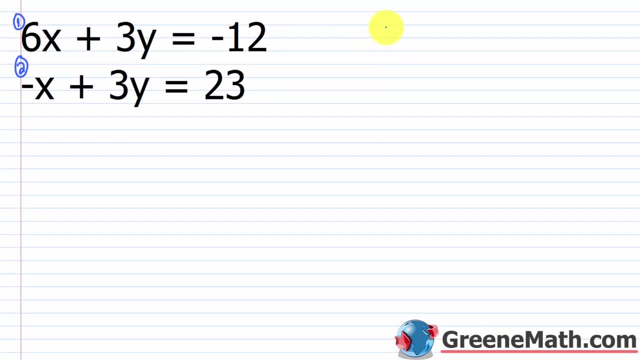 All right, So let's erase everything. So we know that y equals 6.. So the ordered pair would be something comma 6.. So now I can plug in for y in either original equation. Let's go ahead and use equation 2, because it looks a little easier. 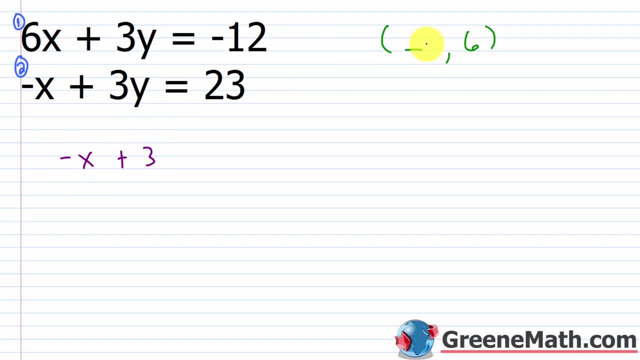 So I would have negative x plus 3 times. plug a 6 in for y equals 23.. So negative x plus 3 times 6 is 18 equals 23.. I can subtract 18 away from each side. I can subtract 18 out of the equation. 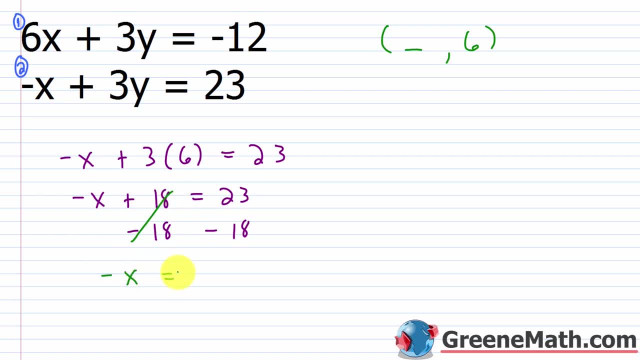 This will cancel. I'll have negative. x is equal to 23 minus 18 is 5.. So, essentially, all I need to do is divide both sides by negative 1 or multiply both sides by negative 1, whatever you want to do. 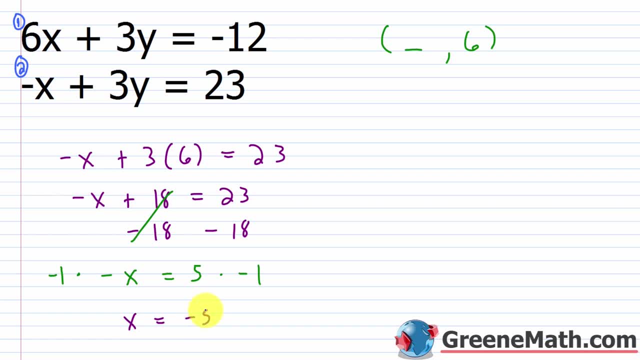 You'll get. x is equal to 5 times negative, 1 is negative 5.. So my x value is negative 5, while my y value is 6.. So the ordered pair: negative 5 comma 6.. So now what I want to do? I want to go into equation 1.. 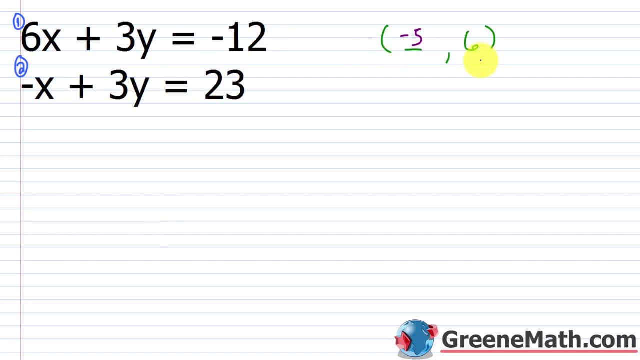 And equation 2, plug in my ordered pair and see if I've got the correct solution for the system. So I've got 6 times for x, I'm plugging in a negative 5 plus 3 times. for y, I'm plugging in a 6 and this should give me negative 12.. 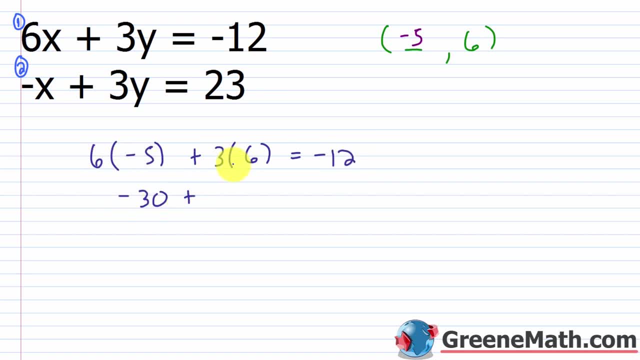 6 times negative. 5 is negative. 30 plus 3 times 6 is 18.. This should give me negative 12 and it does right. You get negative. 30 plus 18 is negative 12 and that equals negative 12.. 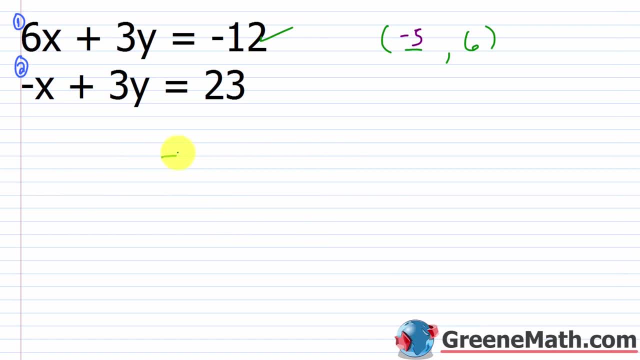 So this one checks out. Now for the next one, we have negative and then I'm plugging in a negative 5. So it's basically the opposite of plug in a negative: 5 plus 3 times y, y is 6, and this should equal 23.. 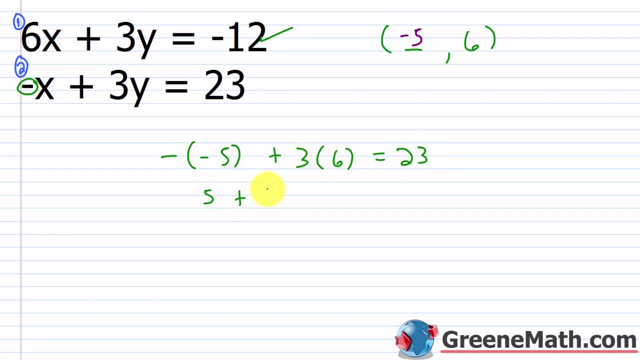 The opposite of negative. 5 is 5 plus 3 times 6 is 18, and this should equal 23, and of course it does. 5 plus 18 is 23, so 23 equals 23, so we verified this one as well. 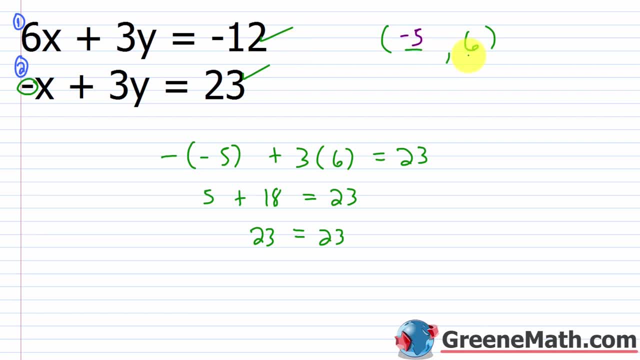 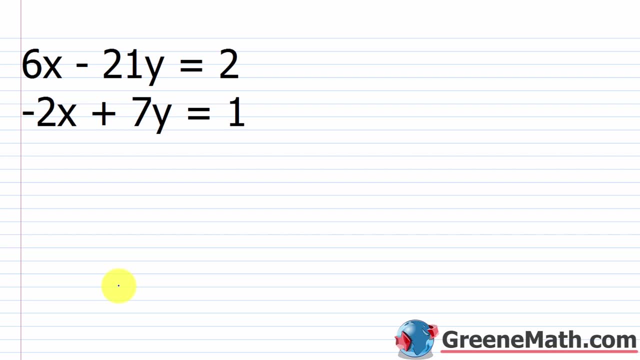 So our ordered pair here, negative 5 comma 6, is the verified solution for this system, Right? so let's take a look at another one. So we have 6x minus 21y, equals 2.. We have negative 2x plus 7y, equals 1.. 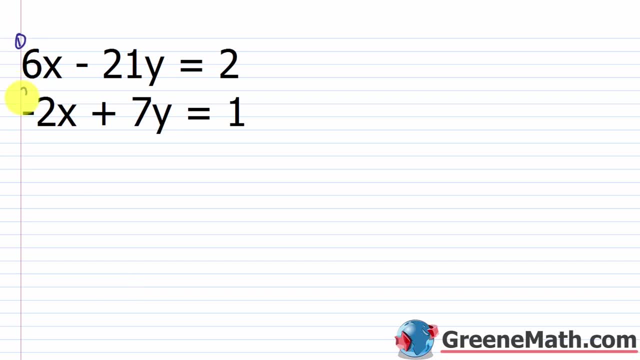 So again, I'm going to label my equations. This is equation 1,, this is equation 2.. None of the variables have a coefficient of 1. None of the variables have a coefficient of negative 1.. So pick whatever you want, whatever you think is easiest for you. 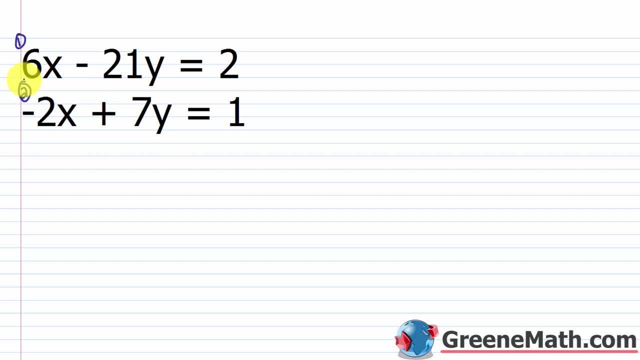 I'm going to go ahead and solve equation 1 for x, the first thing that I see. So if I have 6x minus 21y equals 2, if I'm solving for x, add 21y to each side of the equation. So this is going to cancel. I'll have: 6x is equal to 21y plus 2.. So 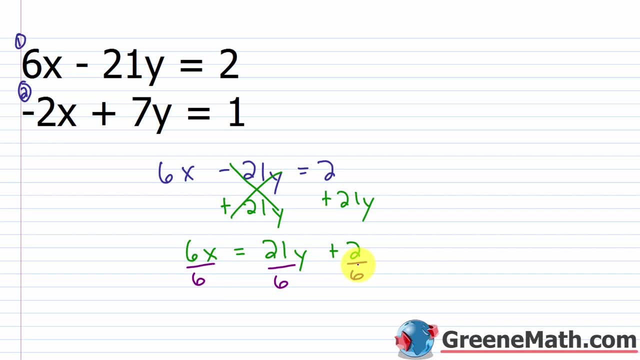 now I'm going to divide both sides of the equation by 6.. This will cancel. I'll have: x is equal to for 21 and 6, they have a common factor of 3.. If I divide 21 by 3,, I get 7.. If I divide 6 by 3,, 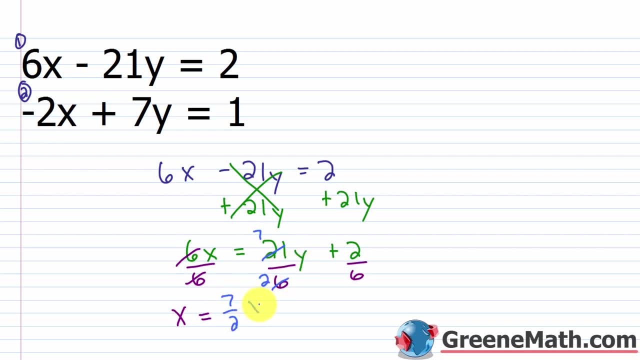 I get 2.. So this is 7 halves times y plus 2 over. 6 is 1 third. So x is equal to 7 halves y plus 1 third. Okay, so let's erase this, And so we got this from equation 1.. Okay. 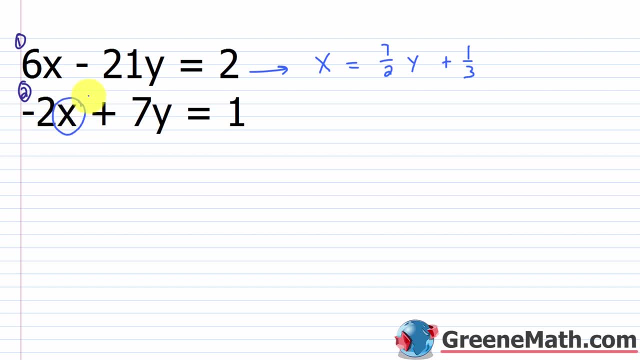 we got this from equation 1.. So I'm going to plug in for x in equation 2. And I'm going to plug this in right: x equals this, So that's going in there. So what are we going to get? We're going to have negative 2 times the quantity 7 halves y plus 1 third. 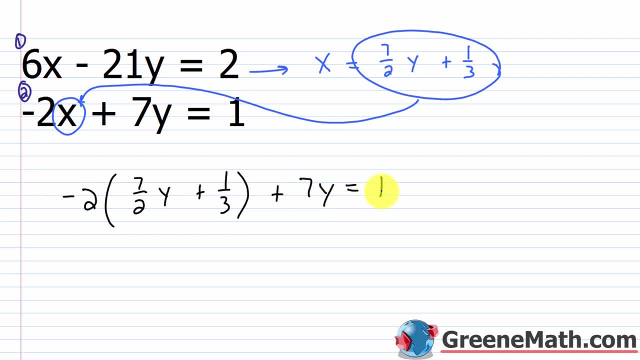 then plus 7y equals 1.. So negative 2 times 7 halves. you can think about negative 2 times 7 halves like that. This would cancel with this and you'd have a negative 7. So this would end up. 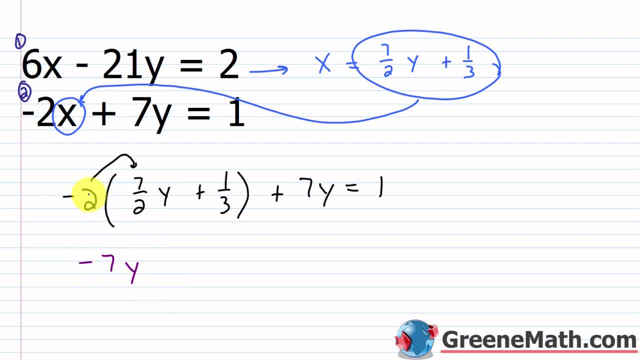 negative 7y And then negative 2 times 1 third would be negative 2 thirds, And then plus 7y equals 1.. Now what happens here? Negative 7y plus 7y is what, That's 0. This cancels. 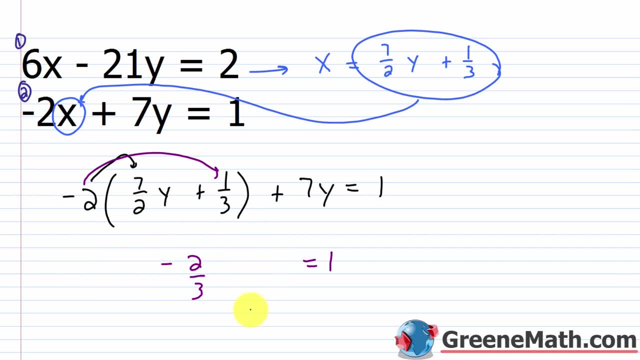 So what am I left with Negative 2 thirds equals 1.. Well, that's not true. That's clearly false. So what happened here? Well, this happens to be a system that has no solution. These are parallel lines. So if your variable drops out when you're doing this, 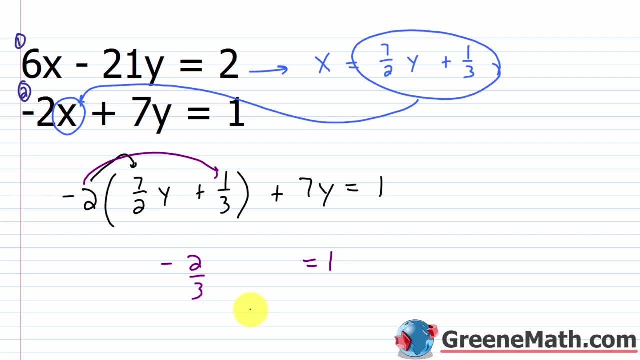 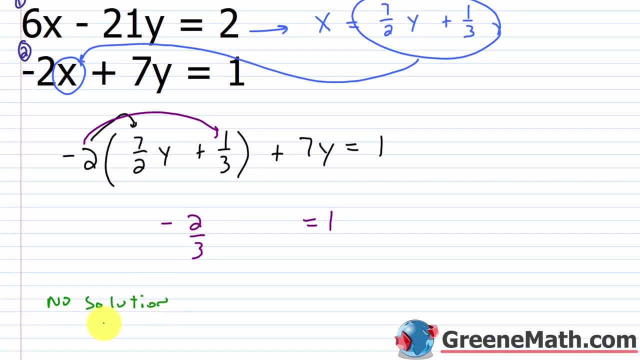 and you end up with a statement that doesn't make sense, like negative 2 thirds equals 1, you have no solution. You have no solution. If the variable were to drop out and you have a true statement, then you have an infinite number of solutions. Now, the easiest way to show this: 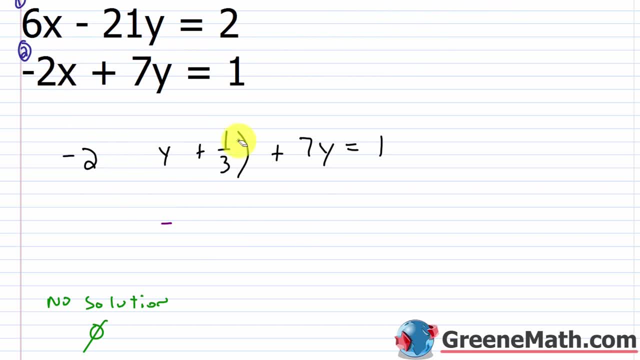 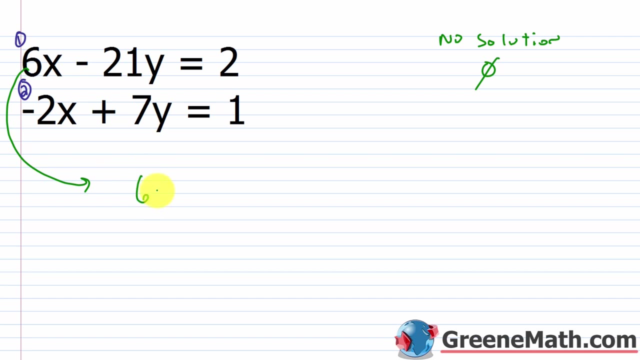 is again to solve each equation for y. If they're each in slope-intercept form, you can see that they are in slope but different y-intercepts And so they're parallel lines. So let's put this over here out of the way. If I solve this for y, 6x minus 21y equals 2.. If I subtract 6x away from 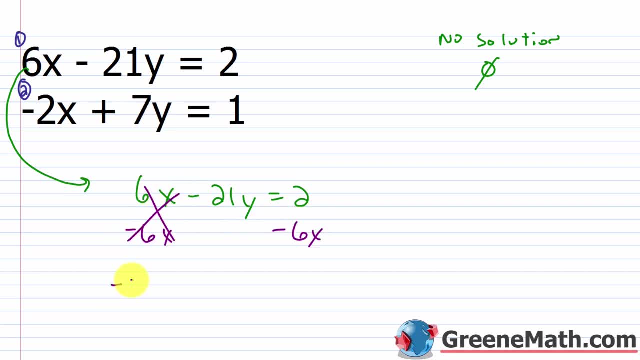 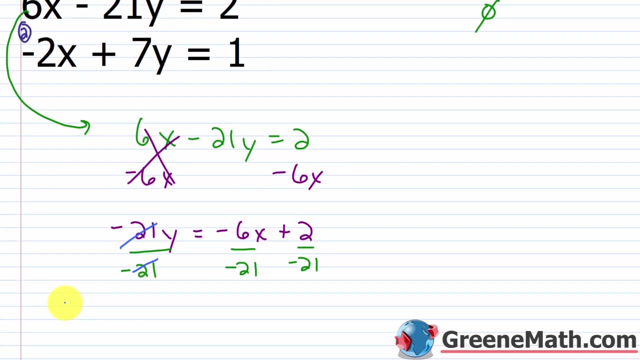 both sides of the equation. this will cancel. I'll have: negative 21y is equal to negative 6x plus 2.. I then want to divide both sides of the equation by negative 21.. And so this is going to cancel. I'll have: y is equal to, So for negative 6 over negative 21,. 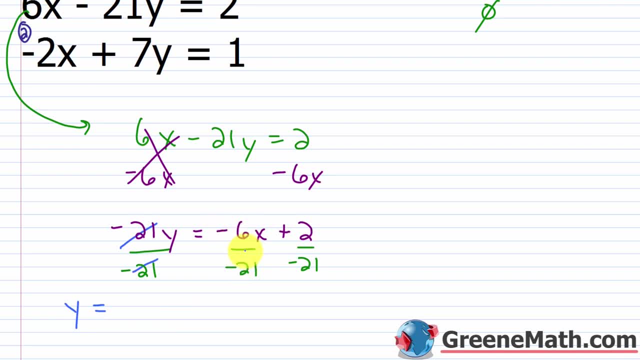 negative over negative is positive 6 over 21,. they're each divisible by 3.. 6 divided by 3 is 2.. 21 divided by 3 is 7.. Then times x And then 2 over negative 21,. we just write minus 2 over 21.. 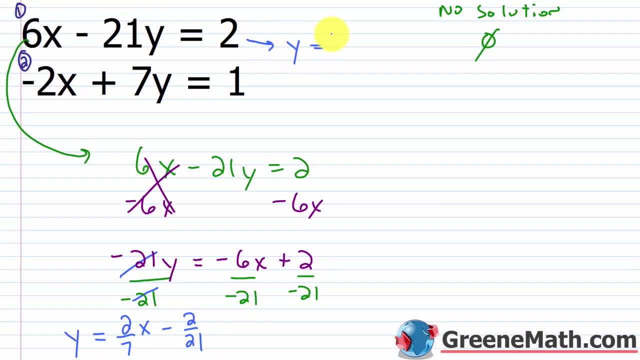 So that's this guy right here: y equals 2 sevenths x minus 2 over 21.. Okay, Let's erase this. And let's now solve this guy for y. So negative 2x plus 7y equals 1.. We'll add 2x to each side of the equation. 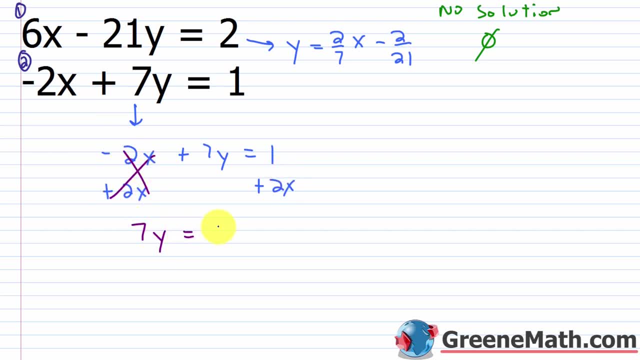 So this is going to cancel. We'll have: 7y is equal to 2x plus 1. Divide both sides of the equation by 7.. So this cancels. You'll have- and I'll write this up here: y is equal to. 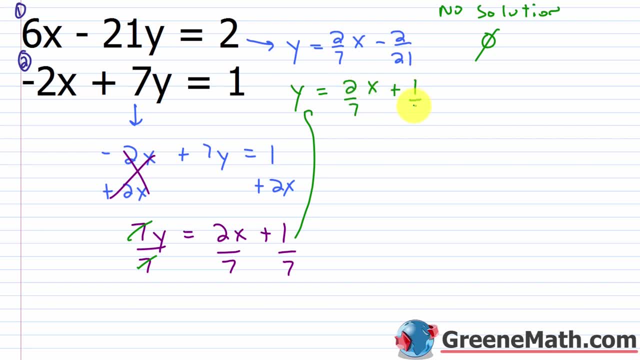 2 sevenths x plus 1 seventh. So let me erase this And I want you to look at this real quick. We know that we have parallel lines when what occurs? We have the same slope but different y intercepts. So in this case the slope is 2 sevenths for each equation. 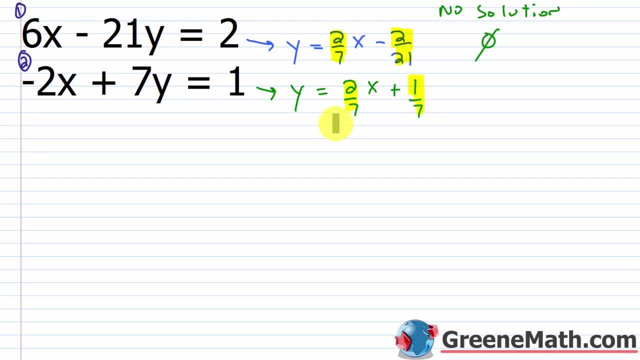 And the y intercepts are different. In equation 1, the y intercept occurs at 0 comma negative 2 over 21.. In equation 2, the y intercept occurs at 0 comma negative 2 over 21.. In equation 2,: 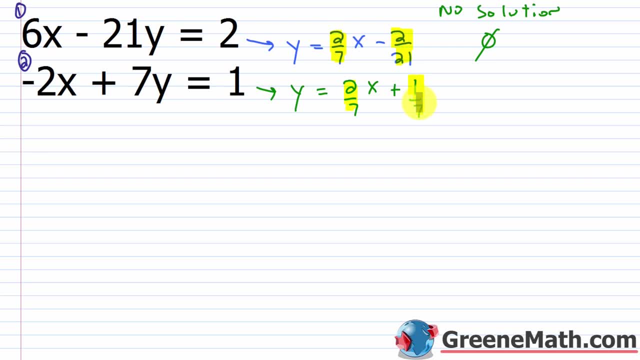 the y intercept occurs at 0 comma negative 2 over 21.. In equation 2, the y intercept occurs at 0 comma negative 2 over 21.. So same slope, different y intercepts, parallel lines never going to intersect. 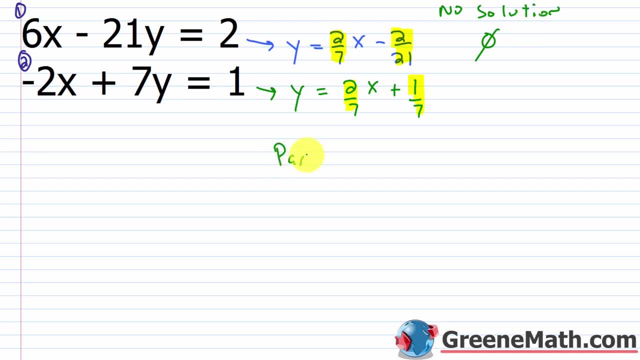 so there's no solution. Okay, these are parallel lines. All right, let's take a look at another one. So we have negative 2x minus 2y equals 6.. And we have 4x plus 6y equals negative 2.. So it looks pretty easy if I solve this guy right here. 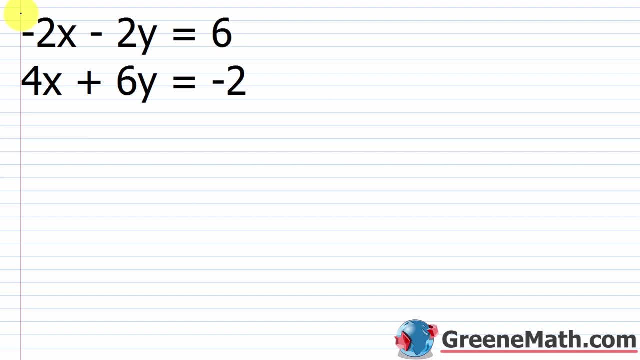 for either x or y. That looks easiest to me. So let's label this as equation 1, and this is equation 2.. And I'll go ahead and solve equation 1 for let's say x, So negative 2x minus 2y equals 6.. Let's go ahead and add 2y to both. 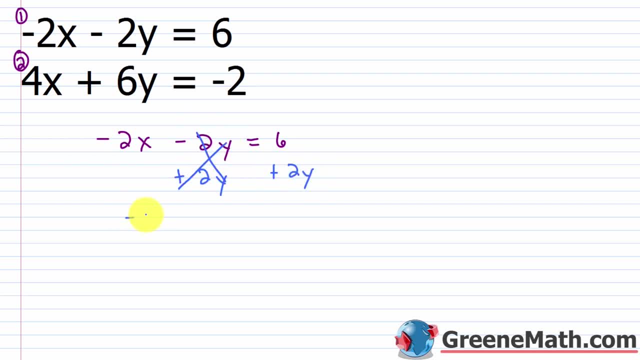 sides of the equation. So that'll cancel. We'll have negative 2x is equal to 2y plus 6.. And as a final step, let's divide both sides of the equation by negative 2.. So that'll cancel. I'll have: x is equal to 2 over negative 2 is negative 1, so negative y. 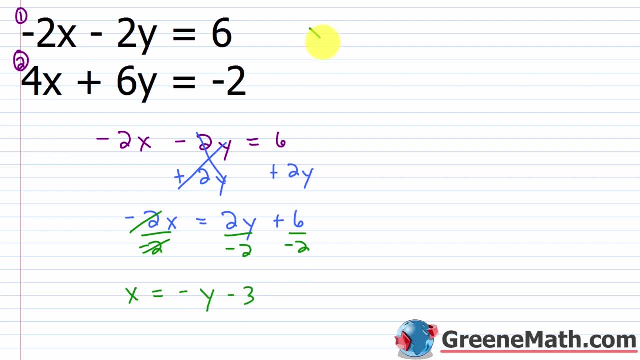 6 over negative 2 is negative 3, so minus 3.. So x is equal to negative y minus 3.. So now, what am I going to do? I'm going to plug in 4x in equation 2. now I found out that x is. 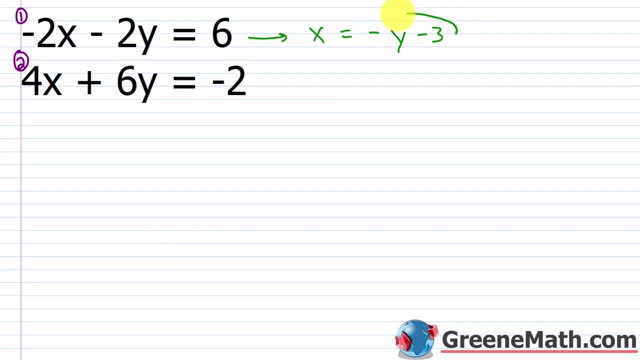 equal to, or x is the same as negative y minus 3, that quantity. So I can plug in for x in the second equation. So 4 times again this quantity here, negative y minus 3, then plus 6y is equal to negative 2.. All right, so 4 times negative y is negative 4y. 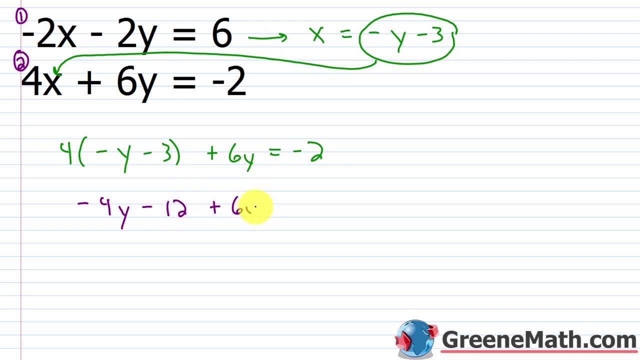 4 times negative. 3 is minus 12, then plus 6y equals negative 2.. All right, so negative 4y plus 6y is 2y, then minus 12 equals negative 2.. And again, if I add 12 to both sides of the equation, that will cancel. We'll have 2y is. 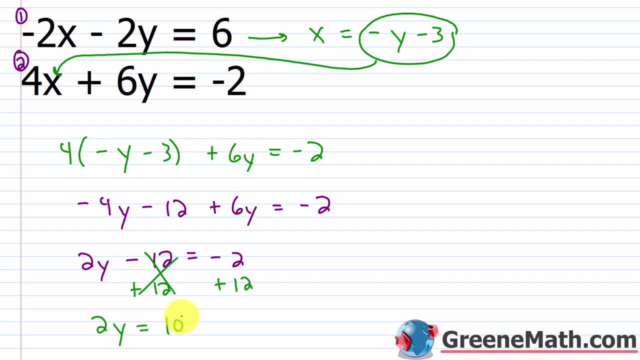 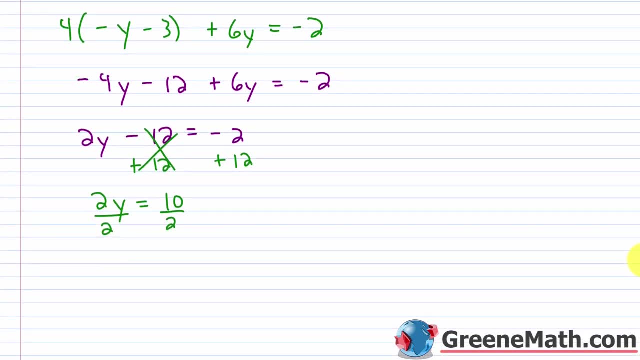 equal to negative. 2 plus 12 is 10.. As a final step, I'm going to divide both sides by 2, and we're going to get that. I'm going to kind of scroll down a little bit. we're in a lot of room, So this will cancel. y is equal to 5.. Let's erase everything. 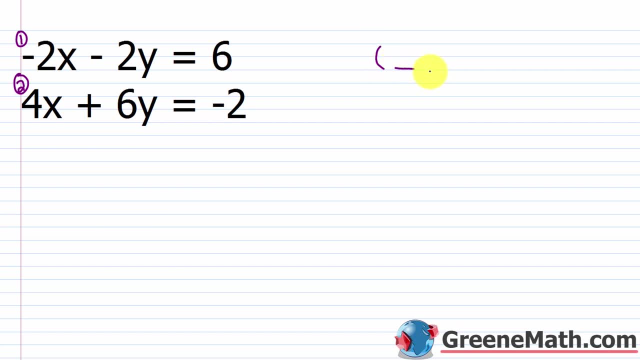 So we say that y equals 5.. So as an ordered pair, something comma 5.. All right, so I'm going to plug in for y in either original equation, Equation 1 or 2, doesn't matter, Let's go ahead and pick equation. 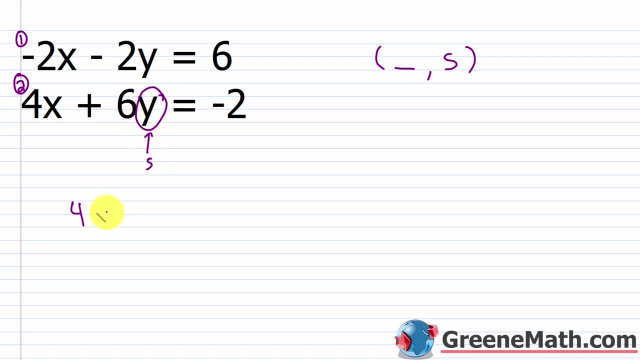 2. So I'm going to plug in a 5 there. So I would have 4x plus 6 times 5 is 30. So plus 30 equals negative 2.. So let's subtract 30 away from each side of the equation. This would cancel 4x is. 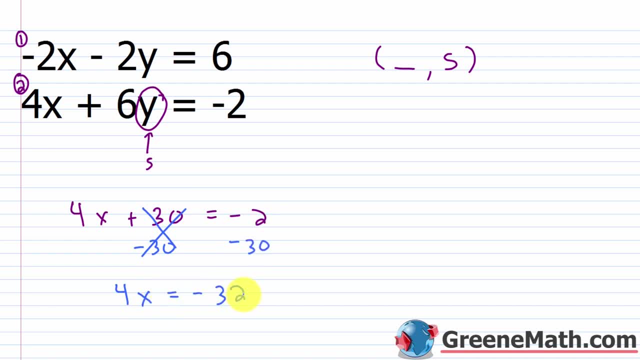 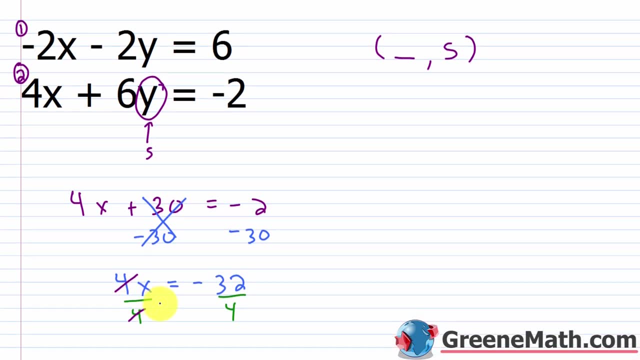 equal to negative. 2 minus 30 is negative 32.. As a final step, let's divide both sides by 4, and this is going to cancel. We're going to end up with: x is equal to negative. 32 over 4 is. 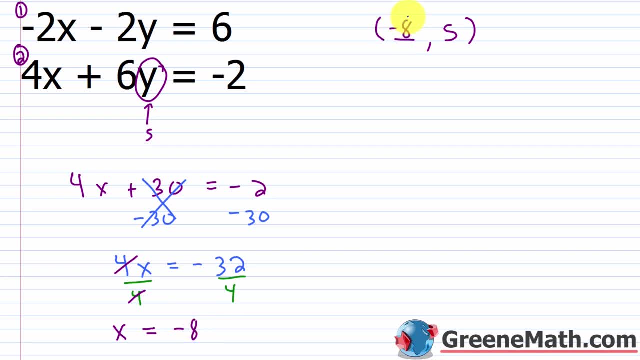 negative 8.. So my x value is negative 8, my y value is 5.. We're getting the ordered pair: negative 8 comma 5.. So let's check this. I'm going to go ahead and plug into each original equation. 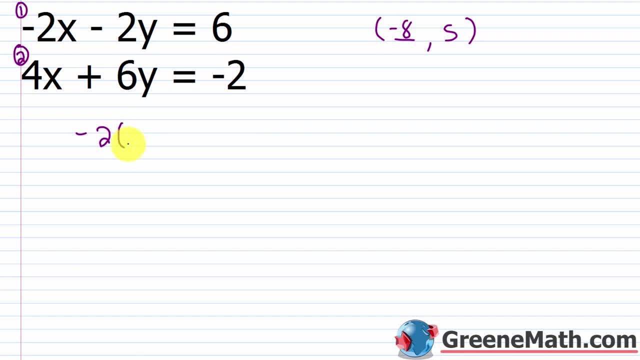 So in equation 1, I have negative 2 times negative 8, that's my value for x, minus 2 times 5, that's my value for y, And this should equal 6.. Negative 2 times negative 8 is 16.. Negative 2 times 5 is negative 10,. 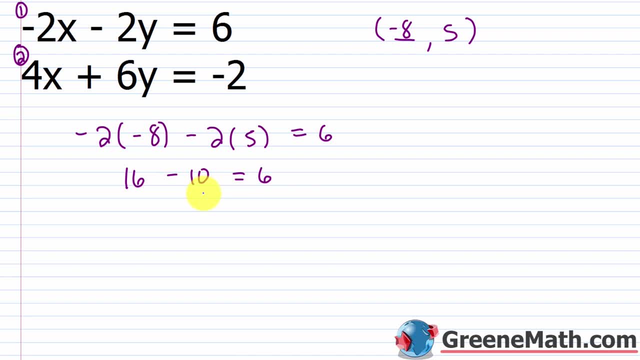 and then we have equals 6.. So 16 minus 10 is 6.. So you get 6 equals 6.. So it works out here In the second equation- remember that's what we used to find x. We know it already works. 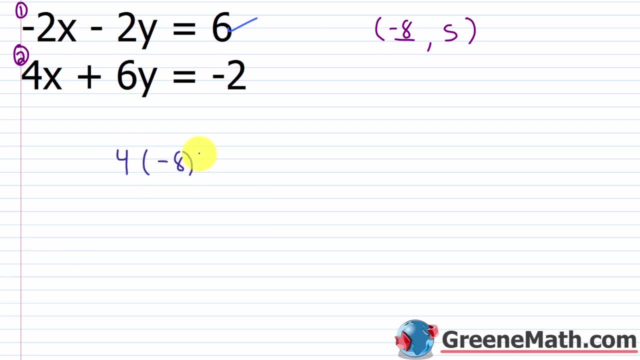 but let's substitute it anyway. So 4 times we have negative 8 for x, plus 6 times we have 5 for y, This should equal negative 2.. 4 times negative 8 is negative 32, plus 6 times 5 is 30. This should equal negative 2,. 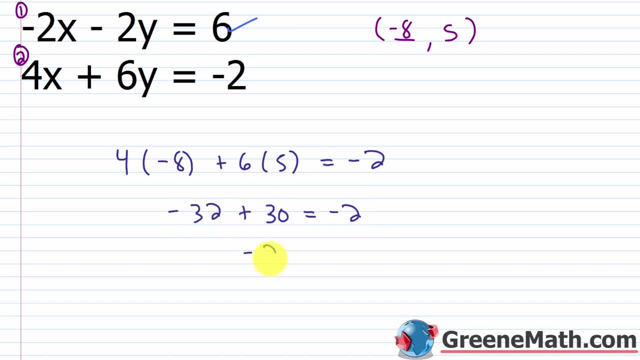 and of course it does Negative 32 plus 30 is negative 2. So negative 2 equals negative 2. So it works out here as well. So we've verified that the ordered pair- negative 8 comma 5, is our solution for this system. 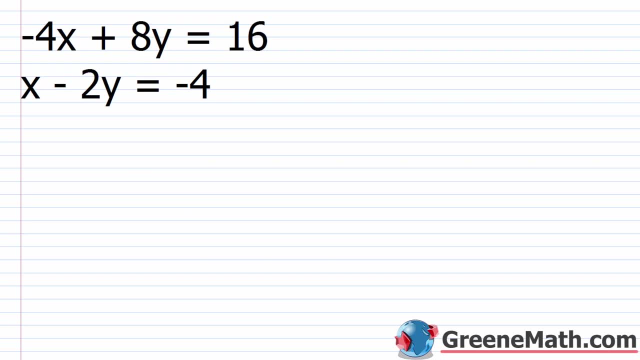 All right, let's take a look at one more problem. So we have negative 4x plus 8y equals 16, and we have x minus 2y equals negative 4.. So I notice that this equation here- and I'm going to label this equation 1 and equation 2,- 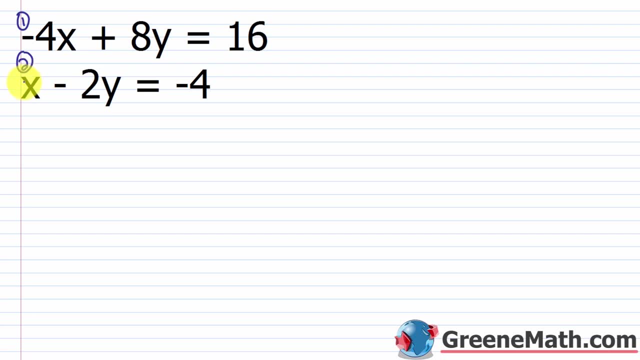 this equation 2 has a coefficient on x, that is 1.. So when that occurs, it's like hitting the lottery You want to solve for that one. I've got to use that because it's easy, So I'm going to say: okay, I have x minus 2y equals negative 4.. I'm going to add 2y to both. 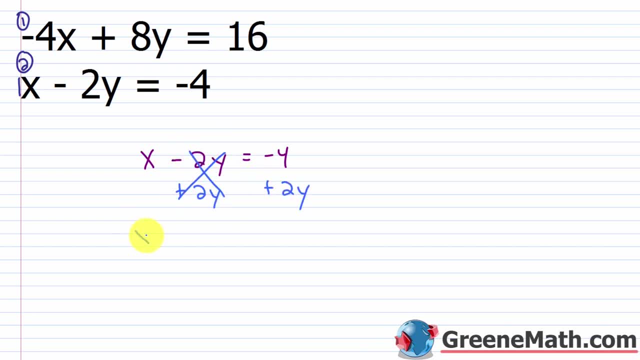 sides of the equation. This will cancel. We'll have x which is equal to 0.. I'm going to add 2y to both sides of the equation. This will cancel equal to 2y minus 4.. So now, if I know what x equals or what x is the same as I can plug in. 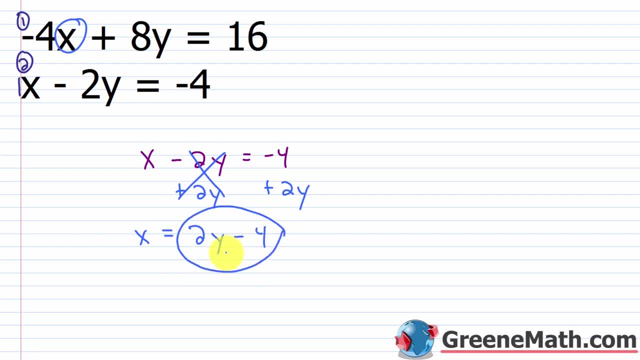 for x in equation 1.. So I'm going to plug this quantity 2y minus 4 in for x there. So I would have what I would have: negative 4 times the quantity 2y minus 4 plus 8y equals 16.. So let 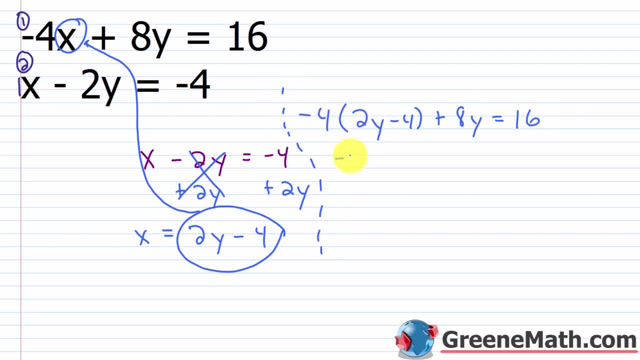 me kind of do this off to the side here. Negative 4 times 2y is negative 8y. Then negative 4 times negative 4 is plus 16. Then plus 8y equals 16.. Negative 8y plus 8y is 0.. This cancels Uh-oh. 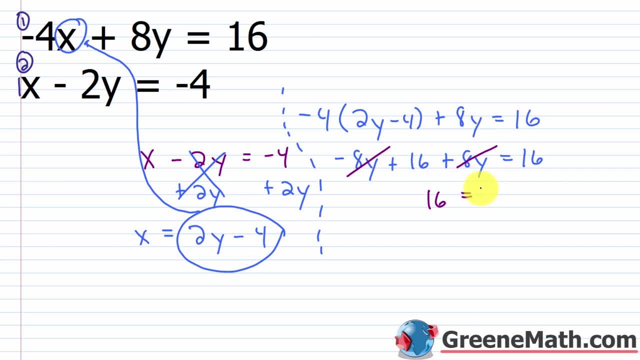 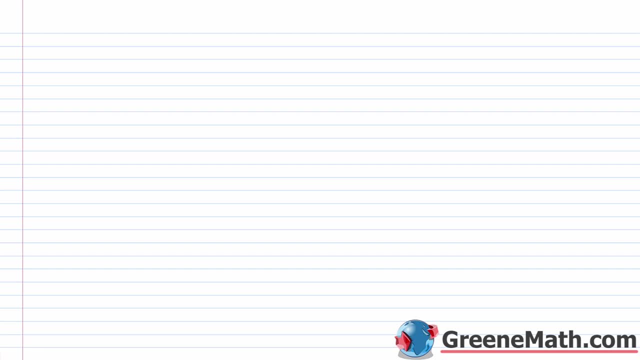 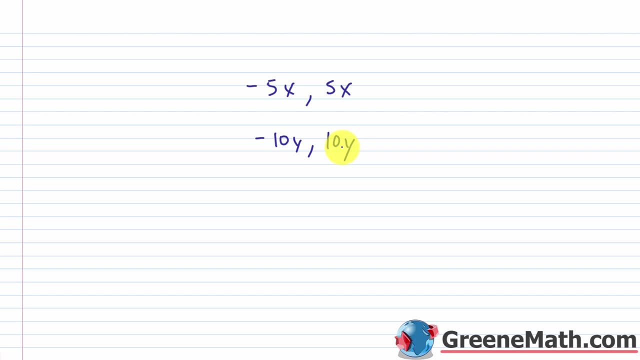 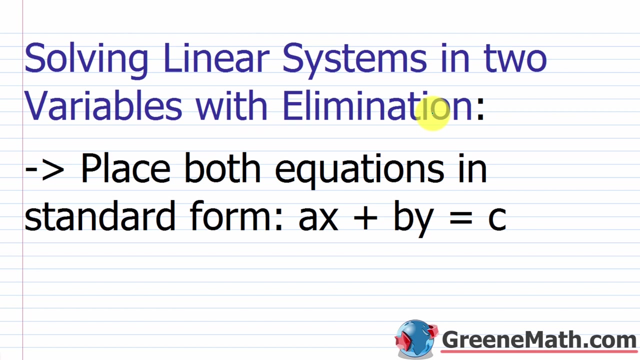 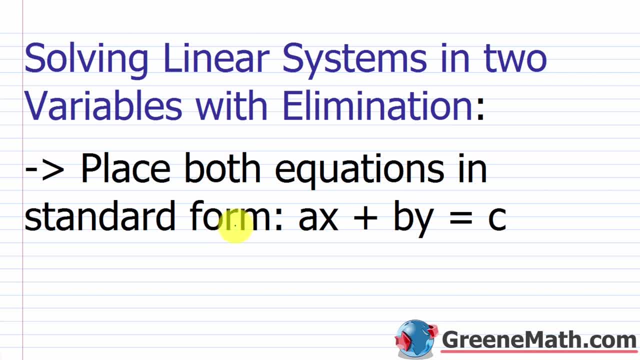 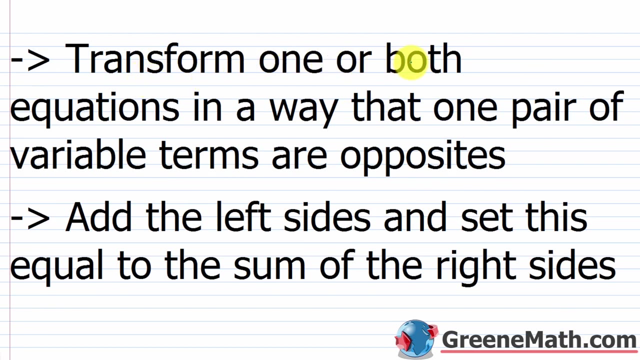 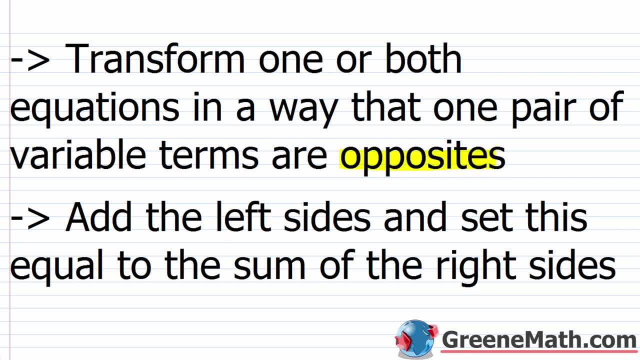 opposites, okay, Opposites. Remember the examples I gave: 5x and negative 5x, or 10y and negative 10y. So you want variable terms that are opposites. Now one of the easier problems this is given to. 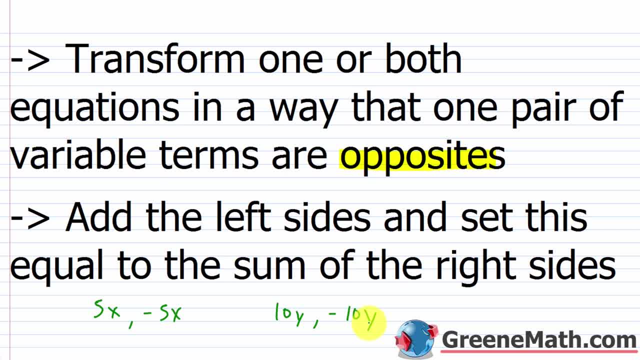 you. you start out that way, One of the harder problems. you've got to transform one of the equations or you've got to transform both of them. okay, And we'll see some examples of that. Now, once this is done, this is where your addition, property of equality, is going to come. 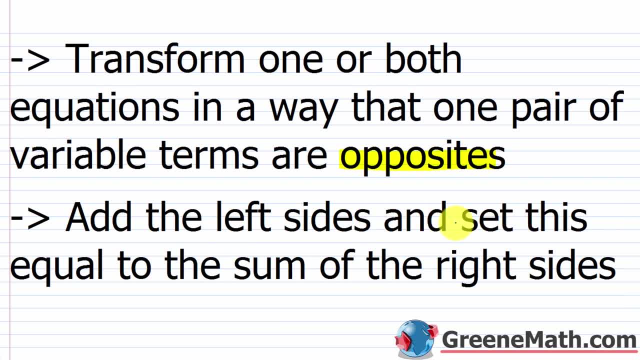 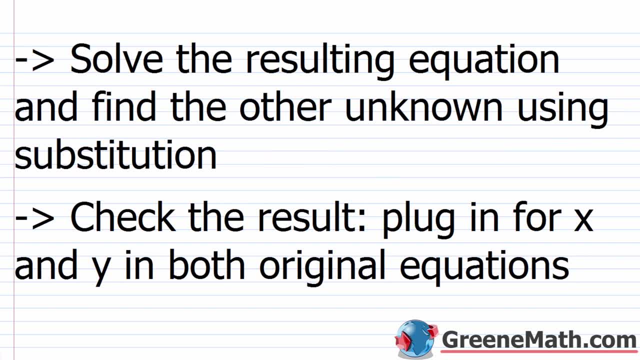 into play. You're going to add the left sides and set this equal to the sum of the right sides, And this will make more sense once we get into the example right. So once you've done your addition step, you will have eliminated one of the variables. So you're left with a linear equation. 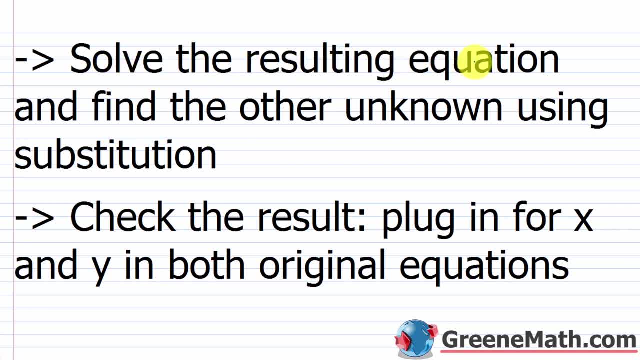 of one variable. So you're going to solve the resulting equation. okay. Once that's done, you'll have x equals some value, or you might have y equals some value, depending on what went on, And then you're just going to find the other unknown, using substitution. So whatever I find, 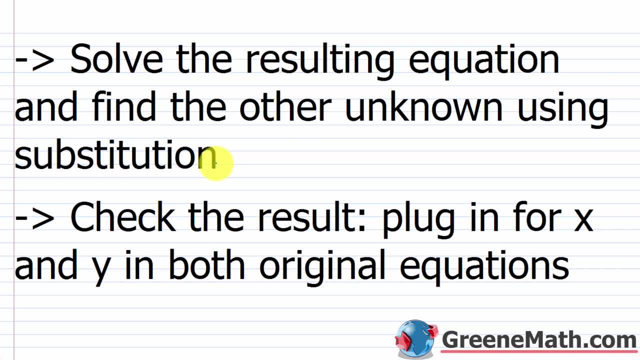 I'm going to plug that back in for that particular variable in one of the original equations I'm going to solve for the other, unknown. Now the last thing and the most important is to check the result. Remember, for you to have a solution for a system, it's got to work in both. 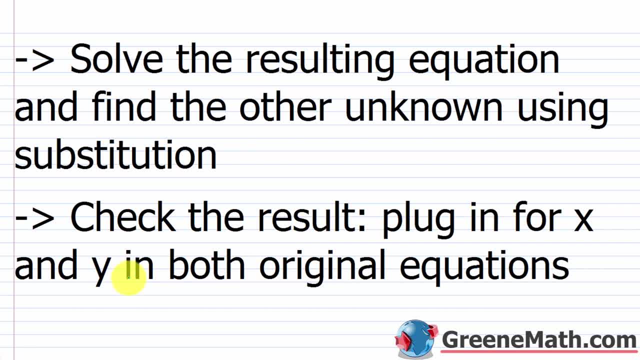 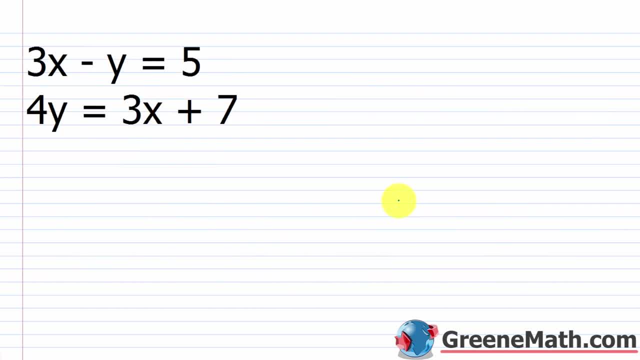 okay, It can't just work in one, So plug in for x and y in both. Let me highlight that in both original equations. All right, so let's go ahead and get started with the first problem. So I have 3x minus y equals 5, and 4y equals 3x plus 5.. 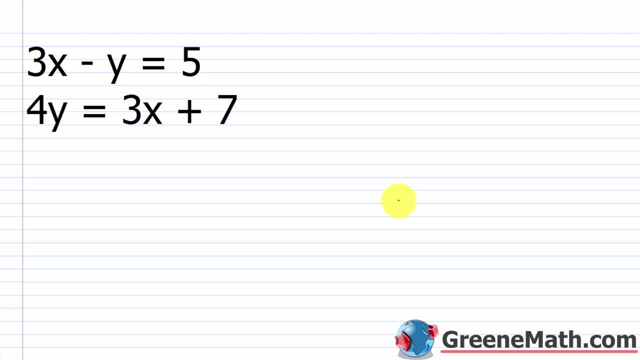 So one thing I like to do, I like to number my equations, just so I can refer to them. So let's say, this is equation 1 and this is equation 2.. So with equation 1, it already follows this format of ax plus by equals c. 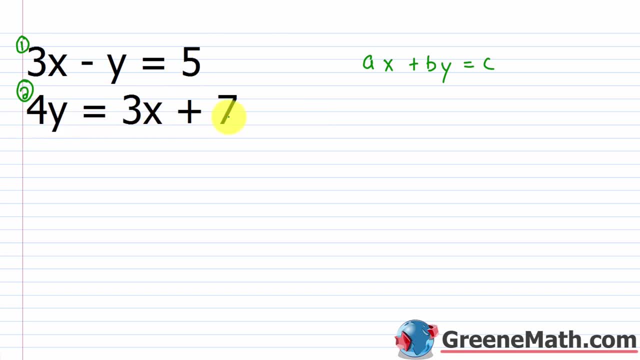 So we don't need to do anything there. With equation 2, not so much, But it's very simple to fix that. All I need to do is subtract 3x from both sides of the equation And I would have negative. 3x plus 4y is equal to 7.. 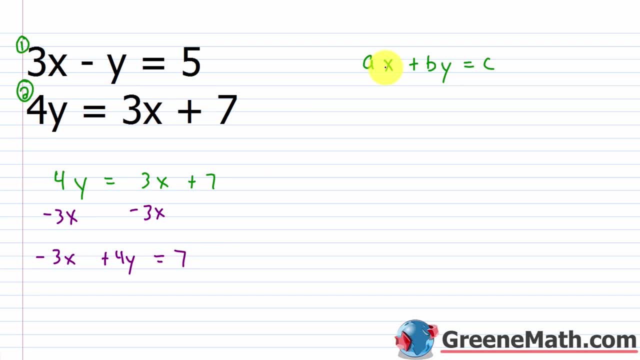 So now it matches this And again we're using the looser definition. So let me erase this real quick And I will drag this up here and just say that we have 3x minus y equals 5. And then this guy negative 3x plus 4y is equal to 7.. 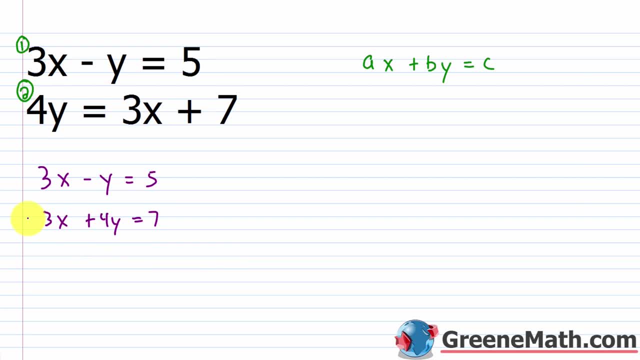 So you can see why we put them both in standard form. It's because we don't want to do anything else. It's because we don't want to do anything else. It's easy to see the values that we have that are lined up on top of each other. 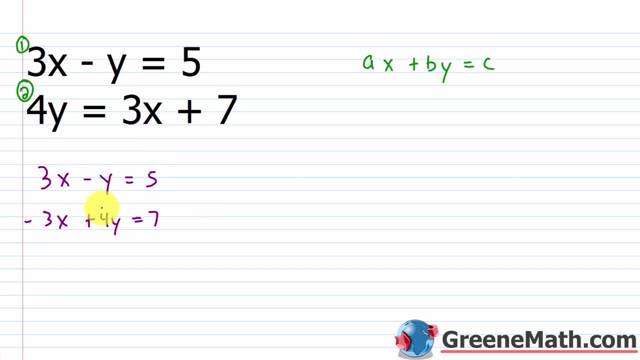 I've got my 3x on top of negative 3x. I've got negative y on top of 4y. I've got 5 on top of 7.. So everything's lined up. In this particular case, we have an easy example. 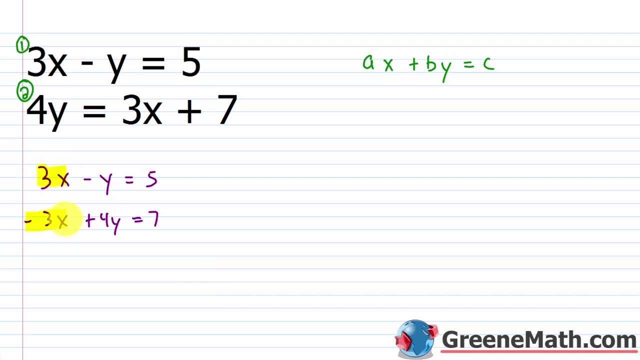 I want you to notice that we have 3x and negative 3x, So we have a pair of variable terms that are opposites. So we don't need to do anything further other than proceed to the step where we add the left side. 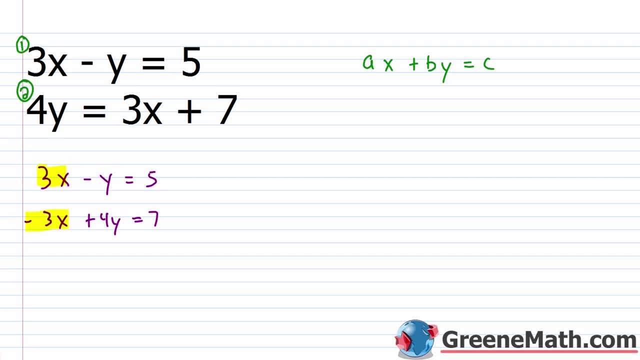 and set that equal to the sum of the right sides. Now, generally we do this vertically, But for the first one I want to do it horizontally. Just to show you something: If I start out with 3x minus y, and this is equal to 5.. 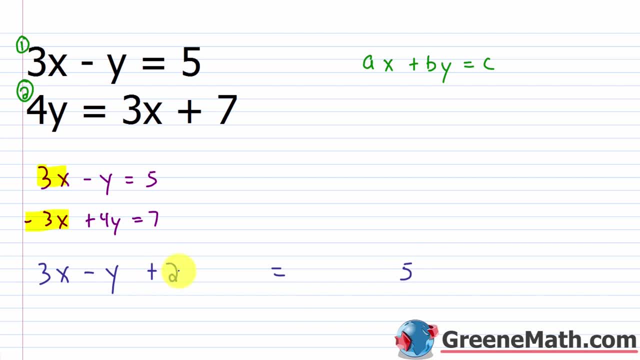 So everybody to this point would understand that it's okay to add 2 over here. as long as I add 2 over here, I added the same thing to both sides of the equation. But where people get confused is if I start doing stuff like this. 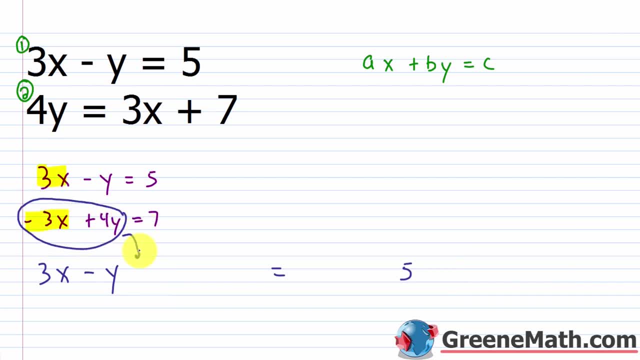 Let's say I add this to this side, So I'm going to add the quantity negative 3x plus 4y. Based on what we've done so far in our algebra coursework, we would expect us to add the same exact thing over here. 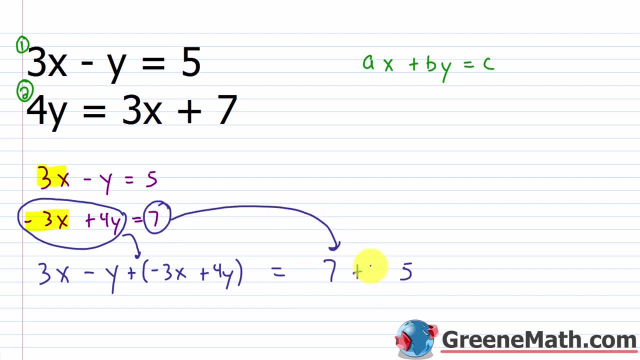 But what I'm going to do is I'm going to add 7 over here. Now you might say: is that legal? Yes, I've added the same thing to both sides of the equation. It doesn't look the same, but I'm told because of this equal sign. 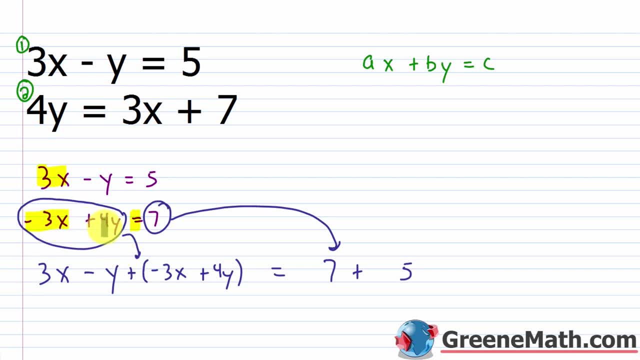 that they are the same. Negative 3x plus 4y is equal to 7, so it's the same as 7.. So if I add this and this, I'm adding the same thing to both sides of an equation And because of the addition property of equality, this is mathematically legal. 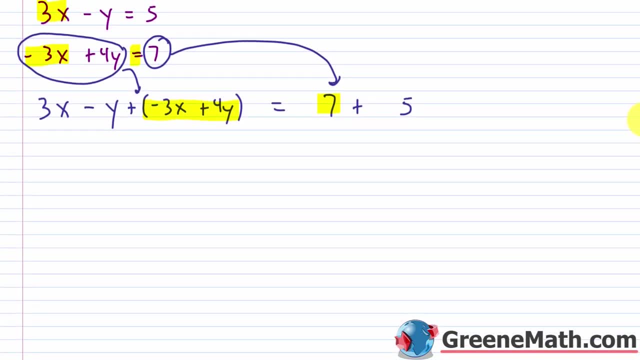 Now let's go ahead and add now and see what we get. So on the left I would have 3x minus y- I'm just going to drop the parentheses here- So minus 3x plus 4y, And this equals. 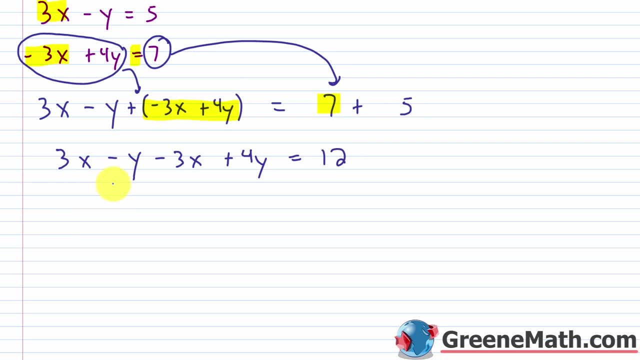 7 plus 5 is 12.. Over here we have that pair of variable terms. You have 3x and negative 3x. Those are going to cancel, And notice how, when they cancel, the x variable is eliminated. Okay, it's gone. 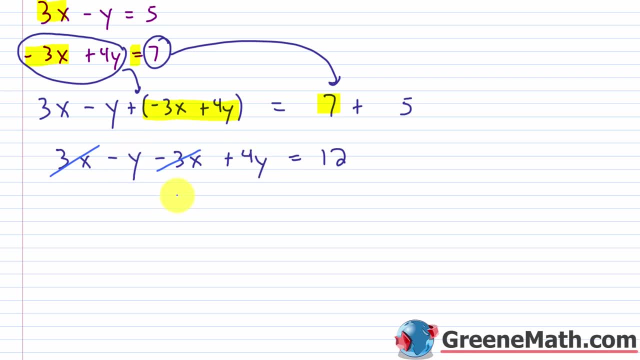 So I'm just left with a variable y. I have negative y plus 4y. That's going to give me 3y, And this is of course equal to 12.. I can now solve my linear equation in one variable. 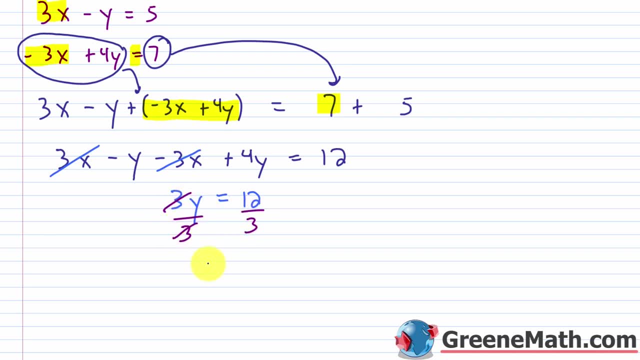 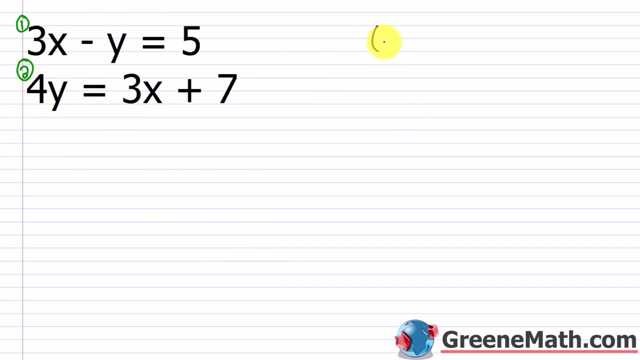 Divide both sides by 3. This will cancel. You'll get: y is equal to 4.. Once you've found that out, just erase everything. So again, y equals 4.. So I would have as an ordered pair something comma 4.. 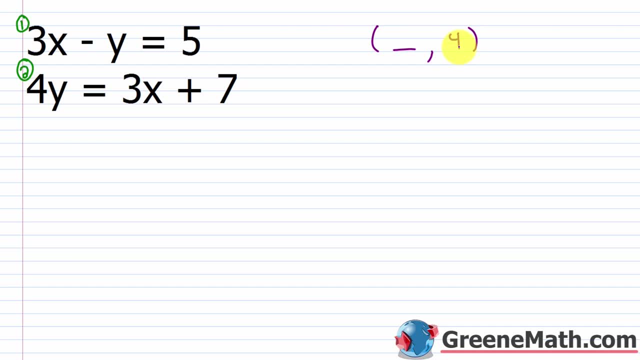 So because 4 is the solution for y in the system, that means it works here and here, okay, in equation 1 and 2. So I can use either equation to find x now. So let's go ahead and go with equation 1, because it seems easier. 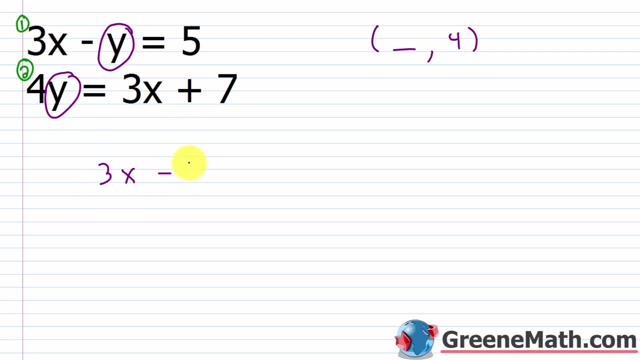 We have 3 times x minus log in a 4 for y and this equals 5.. So what I'm going to do is add 4 to each side of the equation That's going to cancel. I'll have: 3x is equal to 5 plus 4 is 9.. 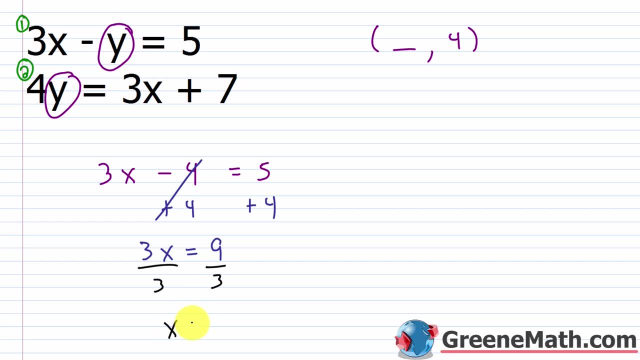 Let's go ahead and divide both sides of the equation by 3. And I'll get: x is equal to 3.. So, as my ordered pair goes, it would be 3 for the x value, comma 4 for the y value. 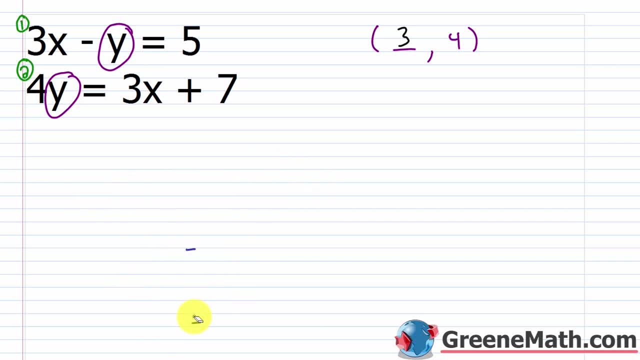 Now the last thing we want to do is make sure that we didn't make a mistake. Remember, this has to work in both equations and this is going to be a solution for the system. So I'm going to take 3 and multiply by x: x is 3.. 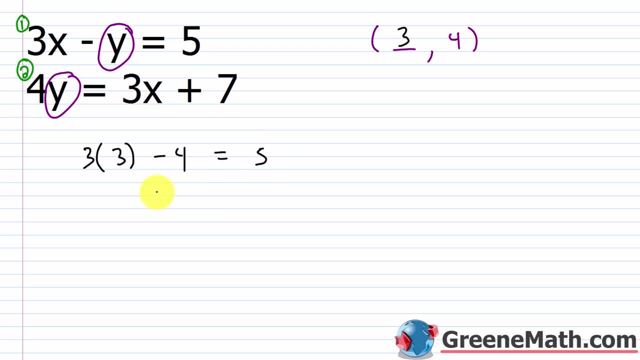 Subtract away 4,, because 4 is y and this should equal 5.. 3 times 3 is 9, 9 minus 4 is 5, you would get 5 equals 5.. So it works out here. 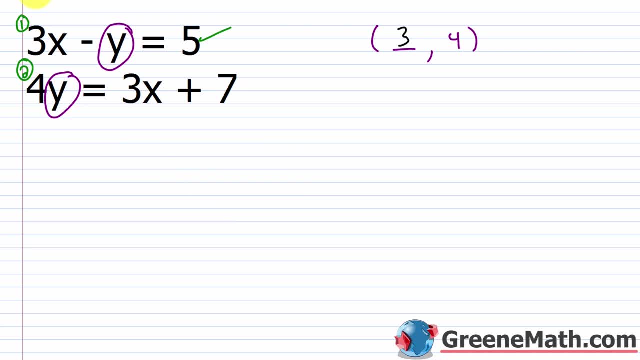 In the second equation, equation number 2, I would have: 4 times y, y is 4, is equal to 3 times x. x is 3, plus 7.. We know 4 times 4 is 16.. 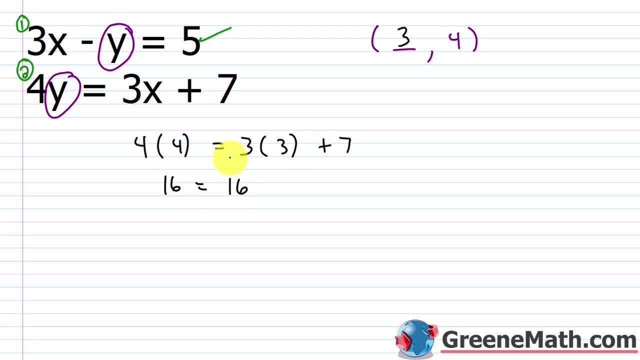 3 times 3 is 9,, 9 plus 7 is 16 as well. So you get 16 equals 16, so it works out here as well. So our solution here is the ordered pair 3, comma 4.. 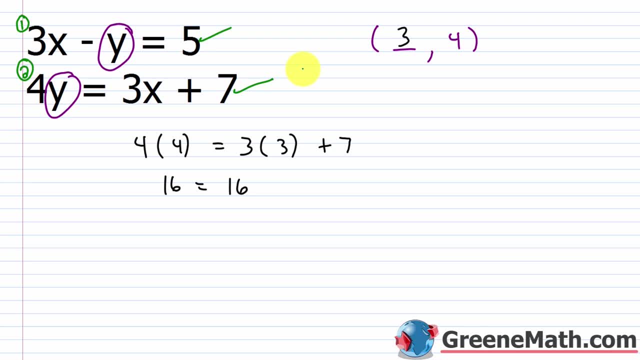 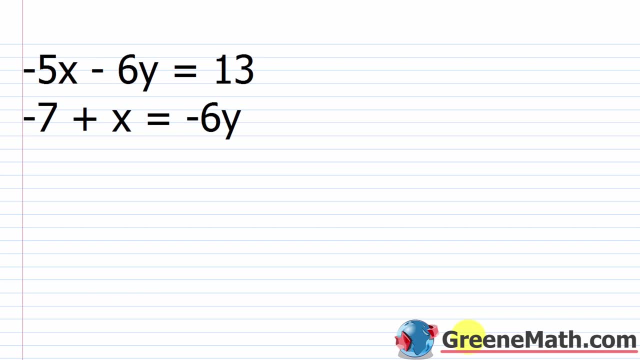 We're getting an x value of 3, a y value of 4.. All right, so let's look at one that's a little bit more challenging. So we have negative 5x minus 6y equals 13,. negative 7 plus x equals negative 6y. 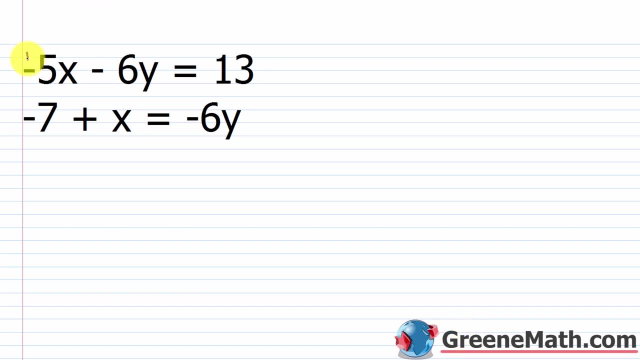 Again. I like to number my equations, Just so I can refer to them. This is equation 1.. This is going to be equation 2.. Now I want them each in standard form, So let me write this again: It's ax plus by equals c. 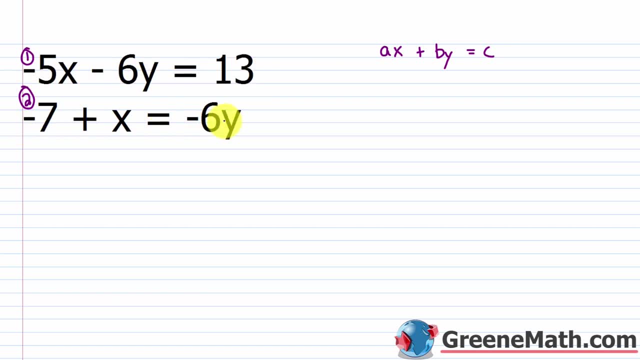 So this one fits the bill. That's okay. This one not so much. What I need to do is subtract x away from each side of the equation, So I would have: negative 7 is equal to negative x minus 6y. And of course I can just flip these around and write: negative x minus 6y is equal to negative 7.. 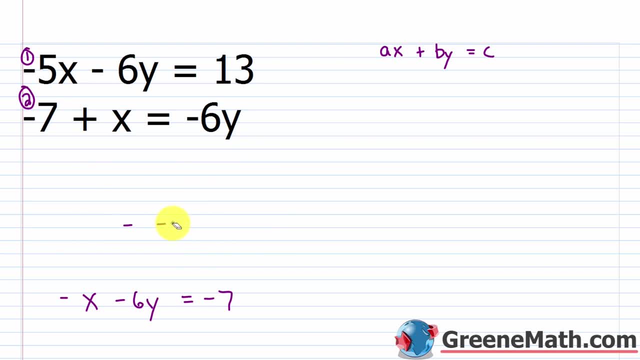 So it matches this. And then let me erase all this, The other guy. equation 1, is negative. 5x minus 6y is equal to 13.. Okay, so now that we've got that, let's take a look at these two equations. 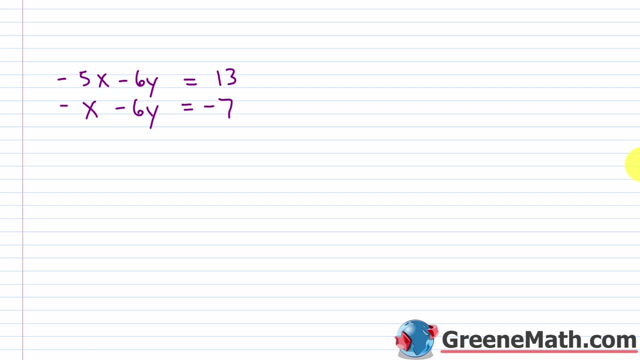 Now, in the last example we were given a nice easy example because we already had a pair of variable terms that were opposites. Here we're not so fortunate. I have negative 5x and I have negative x. Those aren't opposites. 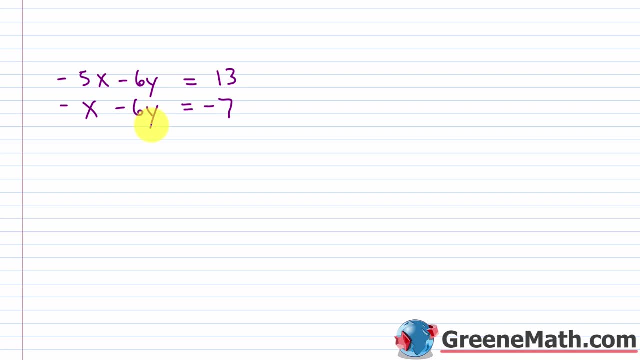 I have negative 6y and negative 6y. Those aren't opposites, But it's still kind of easy, because if I wanted to, I could very easily make these two opposites. All I would need to do is multiply one of the equations by negative 1.. 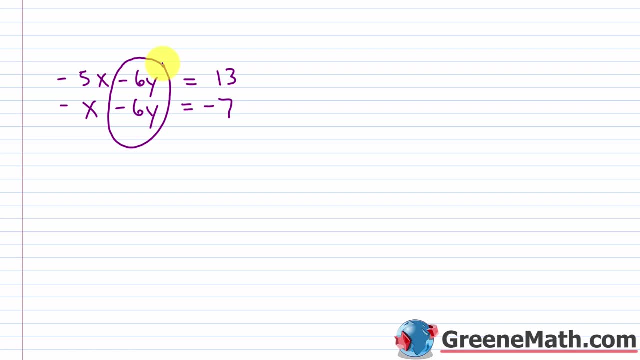 And that negative 6y would become positive 6y. Remember, I can multiply both sides of an equation by the same non-zero number. I can just take this equation here and I can multiply both sides by negative 1. And what I'd get is negative 1 times negative 5x is 5x. 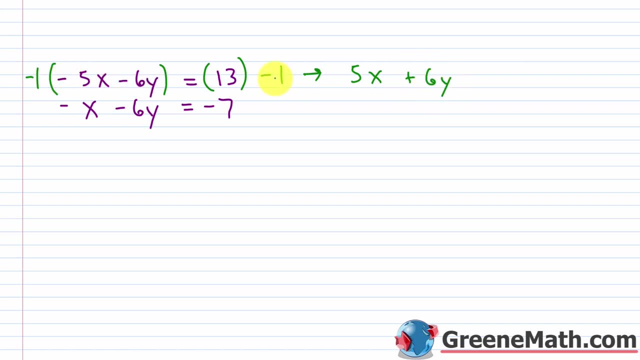 Negative 1 times negative, 6y is 6y. Negative 1 times 13 is negative 13.. So equals negative 13. And this equation stays the same. So we have negative x minus 6y equals negative 7.. 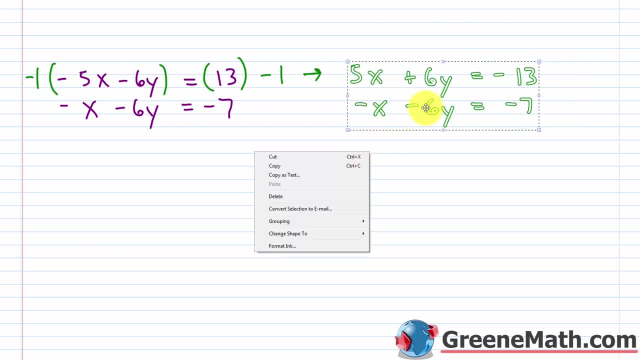 Now let me drag this down here. What you can see is you have 6y and negative 6y. Those are now opposites. So when we sum the left sides and set that equal to the sum of the right sides, that variable is going to drop out. 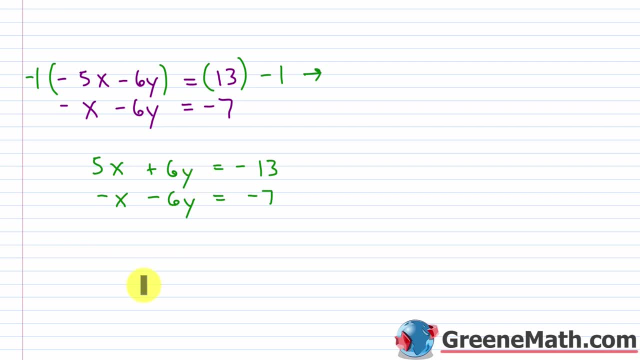 So let's go ahead and do that. So we want to add the left sides together. Set this equal to the sum of the right sides. Now, generally we do this vertically. In the last example I did it horizontally, just to show you. 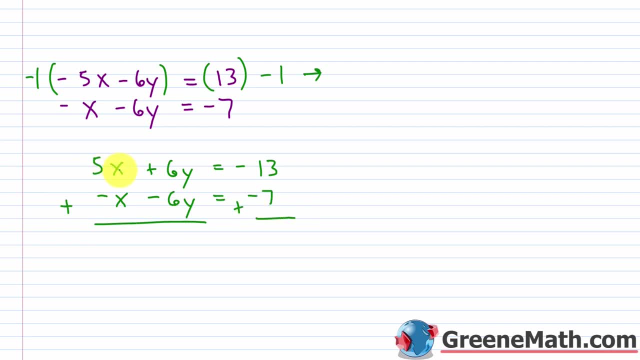 So you just put a plus sign out here And a plus sign out here. So 5x minus x is 4x, 6y minus 6y is 0y. It's just eliminated, So you can line this out. 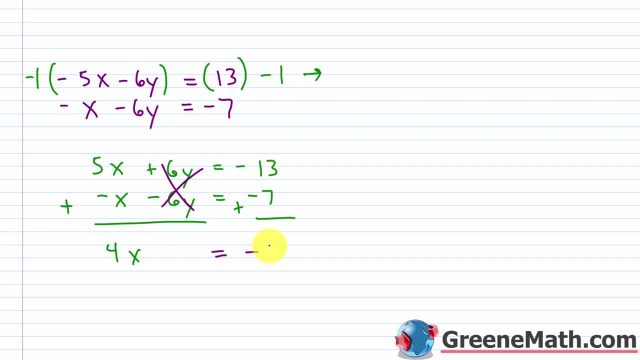 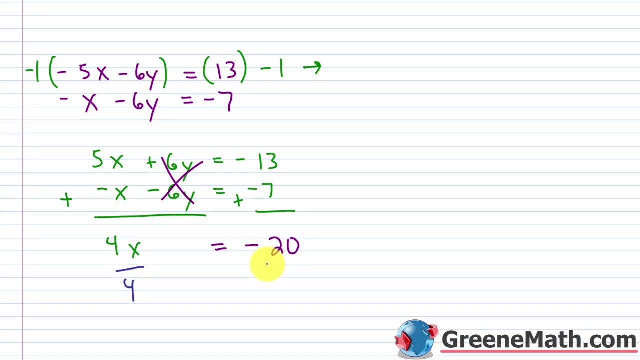 And this is equal to negative 13 minus 7. This is negative 20. So I have: 4x is equal to negative 20.. Of course, to solve for x, I divide both sides by 4. And I get: x is equal to negative 5.. 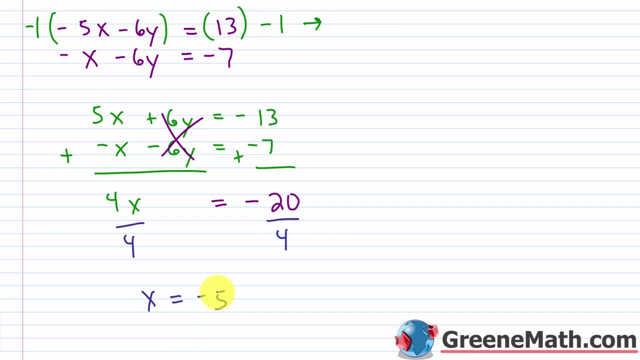 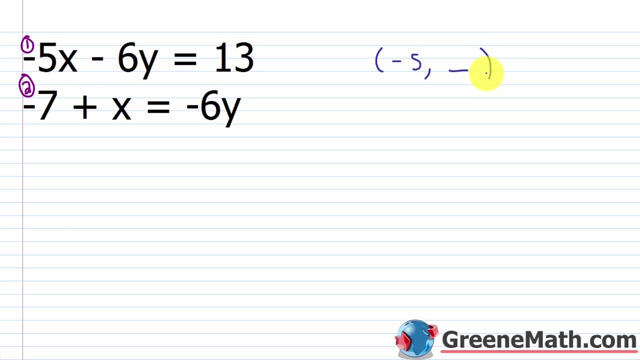 So at this point again, I can erase everything. I just need my two original equations. All right, so we know x equals negative 5.. We don't know the value for y yet, So I'm going to plug a negative 5 in for x, either in equation 1 or equation 2.. 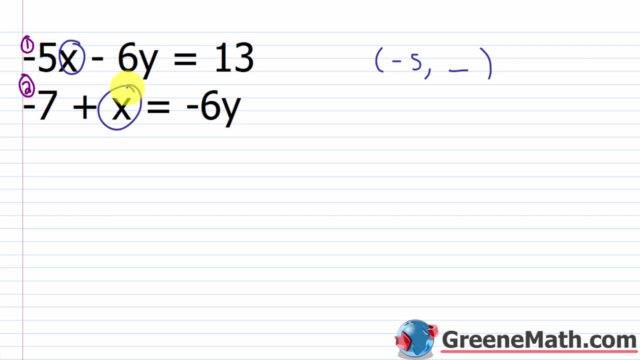 It looks way easier to do it with equation 2. So let's do that, So we would have negative 7 plus a negative 5. And this equals negative 6y Negative 7 plus negative 5 is negative 12.. 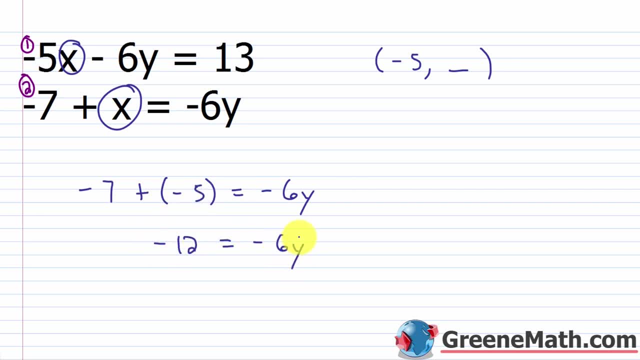 So you'd have: negative 12 is equal to negative 6y. We would divide both sides of the equation by negative 6.. This would cancel. You'd have y is equal to 2.. So x is negative 5, y is 2.. 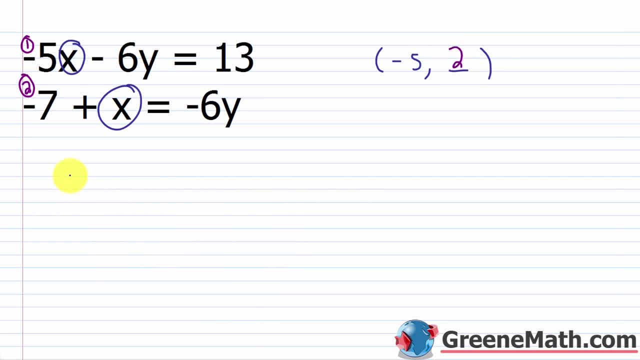 All right, let's erase everything. Let's go ahead and check. So we would have negative 5 times plug in a negative 5 for x, minus 6 times plug in a 2 for y, And this equals 13.. 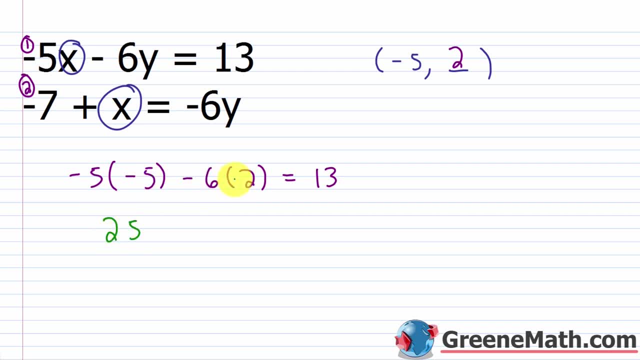 So negative 5 times negative, 5 is 25.. Negative 6 times 2 is negative 12.. And then this equals 13. We know, 25 minus 12 is 13. You would get 13 equals 13 here. 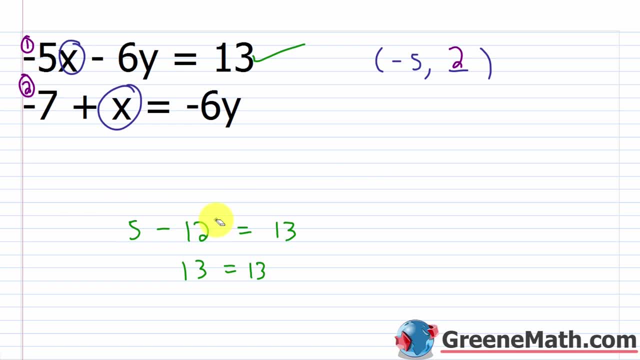 So it checks out here All right. in the next one, equation number 2,, we've got negative 7 plus for x, I've got negative 5. And this should be equal to negative 6 times 2.. Negative 7 plus negative 5 is negative 12.. 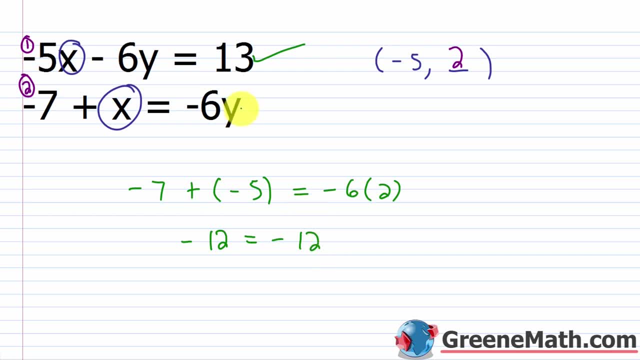 And this equals negative 6 times 2 is negative 12 as well, So it works out here also. So this ordered pair- negative 5 comma 2, or an x value of negative 5, a y value of 2, is our solution for the system. 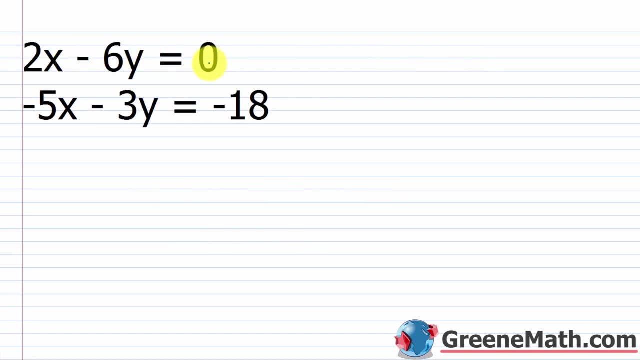 All right, for the next one we're going to look at: 2x minus 6y equals 0. And then negative 5x minus 3y equals negative 18.. So again I like to number my equations. This is going to be equation 1.. 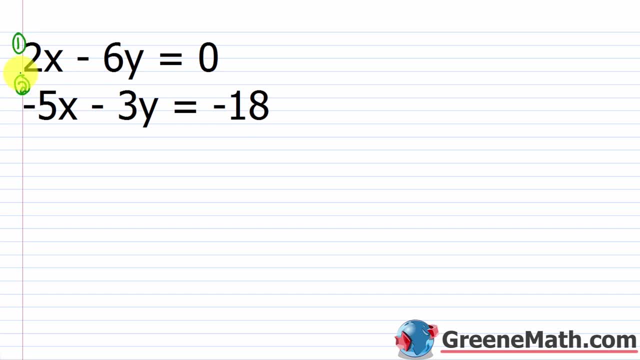 This is going to be equation 2.. Now we want our equations to be in standard form. So ax plus by equals c. This one's in standard form, So is this one. So we're good to go there. Now I want one pair of variable terms to be opposites. 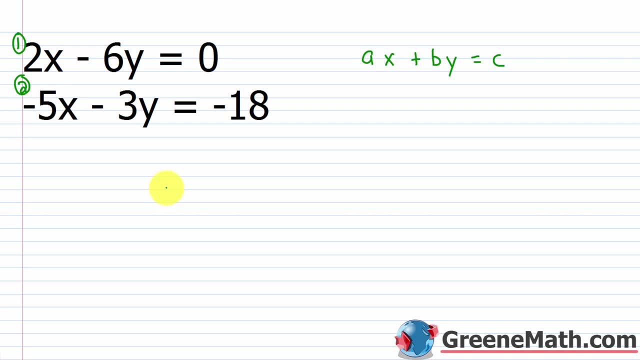 Don't have that. I have 2x and negative 5x, I have negative 6y, negative 3y. So, looking at it, what's the easier option? Do I want to target my x variable or my y variable? 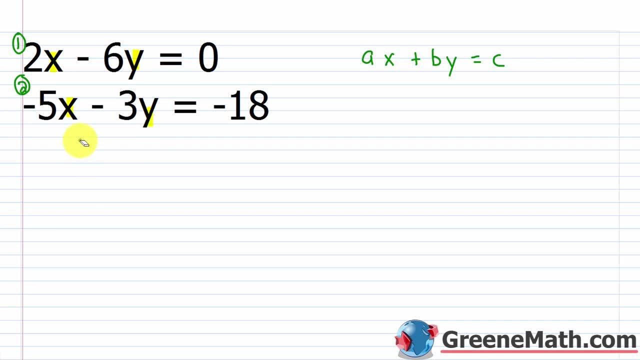 Well, it looks like to me it's easier to target y. The coefficient of y here is negative 6.. The coefficient here is negative 3.. So what I can do is I can multiply equation 2 on both sides by negative 2.. 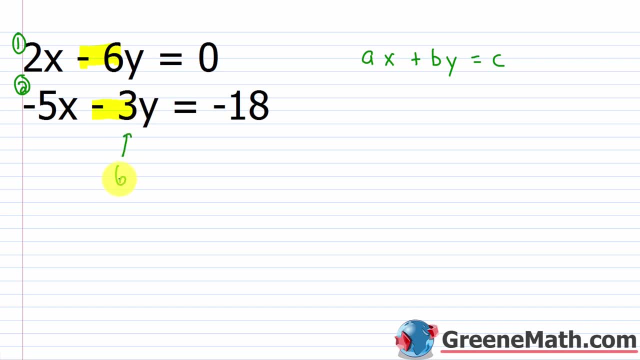 And what that's going to do is give me a value of positive 6 here. So if I have positive 6y here and negative 6y here, those are now opposites. So let's go ahead and crank that out. So for equation 2, I have negative 5x minus 3y equals negative 18.. 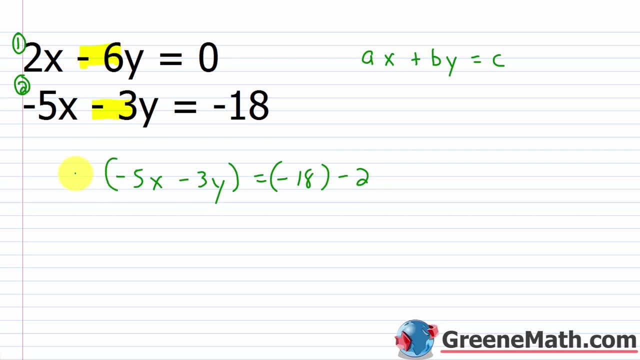 And I'm going to be multiplying both sides by negative 2.. So negative 2 times negative 5x is 10x. Negative 2 times negative 3y is plus 6y, And this equals negative 18 times negative 2, which is 36.. 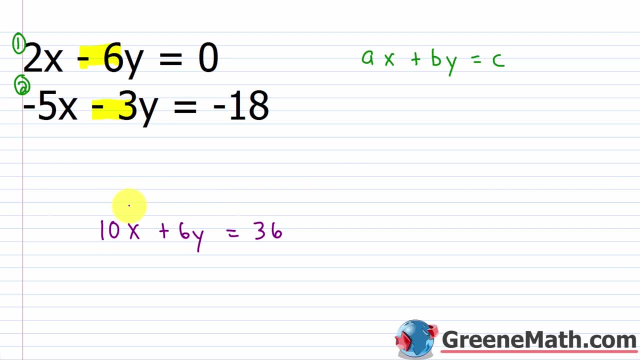 So now that that's done, let me write equation 1 on the top of this. So 2x minus 6y equals 0. So now we're at our step where we can add the left sides together, Set this equal to the sum of the right sides. 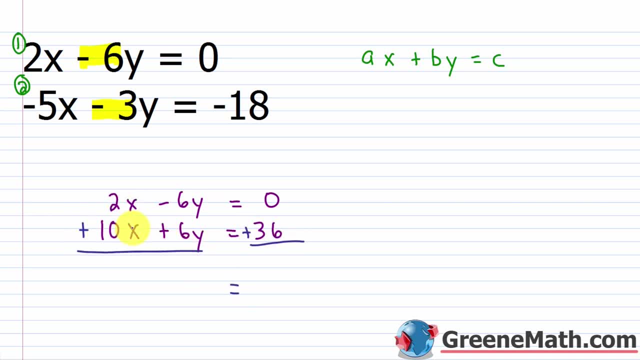 So we're going to add here, add here. So 2x plus 10x is 12x. Negative 6y plus 6y is 0y or just 0. This will be eliminated. 0 plus 36 is 36.. 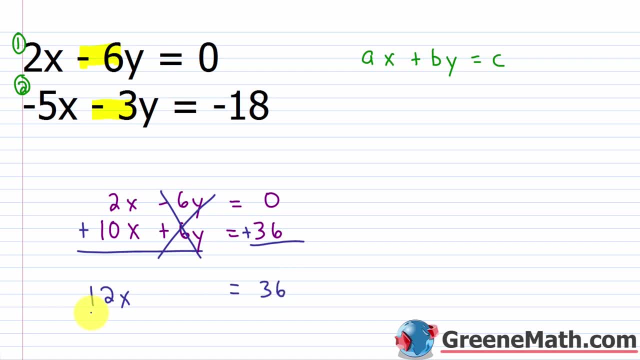 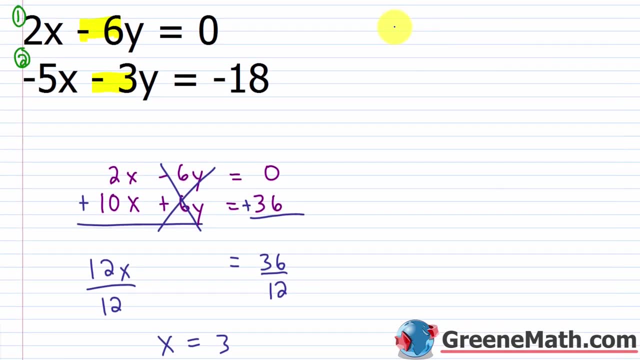 So you get 12x equals 36.. Of course, you can divide both sides by 12. And you'll get x is equal to 3. So let's erase that. As an ordered pair, 3 will be the x value. 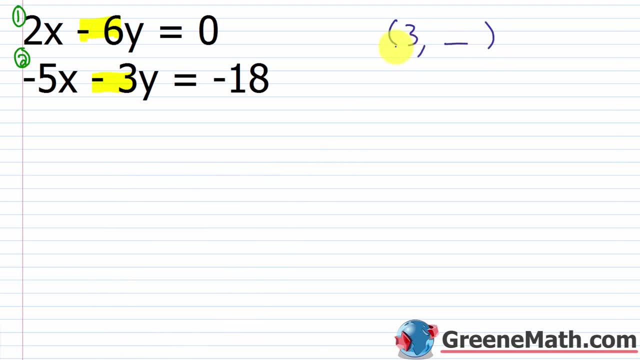 Again, we don't know the y value yet, So I can plug a 3 in for x in equation 1 or 2.. Doesn't matter, Let's just go ahead and plug it in for equation 2.. So I'd have negative 5 times 3 minus 3y equals negative 18.. 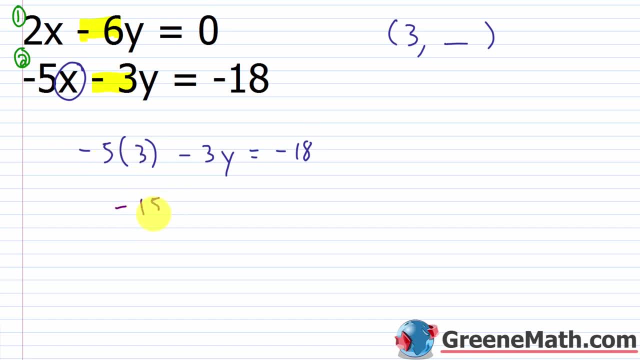 I'm going to multiply negative 5 times 3.. That's negative 15 and minus 3y equals negative 18.. If I add 15 to each side of the equation, that would cancel. I'll have negative. 3y is equal to negative 18 plus 15 is going to give me negative 3.. 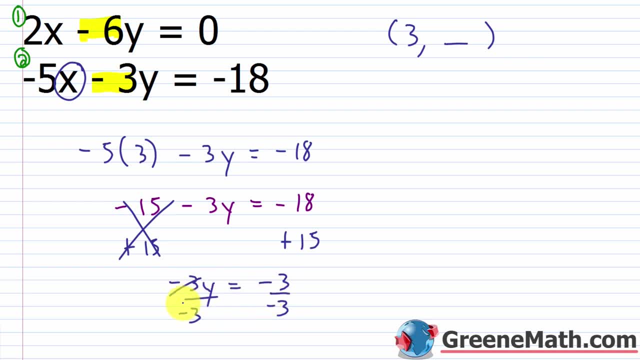 I would divide both sides of the equation by negative 3.. This will cancel. I'll have: y is equal to 1.. So x is 3.. y is 1.. So let's go ahead and check this guy. So in the first equation, equation 1, we'd have 2 times my x value is 3 minus 6 times my y value is 1.. 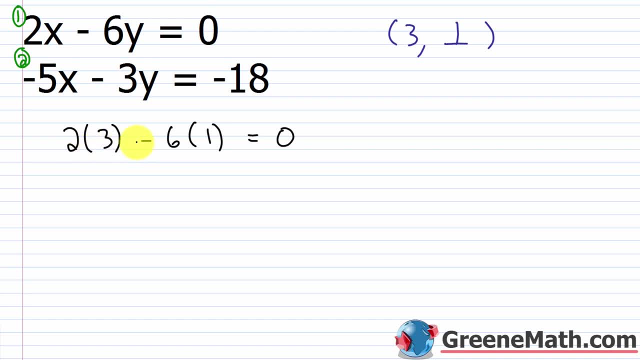 And this should equal 0.. Of course, this would be 2 times 3, or 6 minus 6 times 1, which is 6.. 6 minus 6 is obviously 0.. You would get 0 equals 0.. 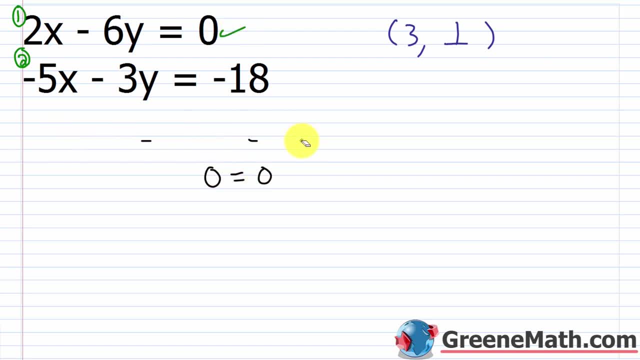 So yeah, it works out here. In the second equation, equation 2,, you would have negative 5 times x. Again, x is 3 minus 3 times y, y is 1. This should equal negative 18.. Negative 5 times 3 is negative 15.. 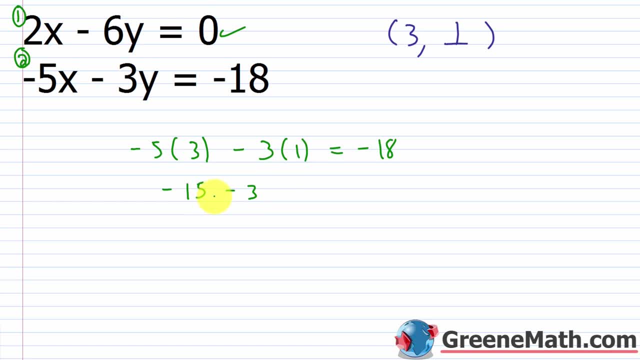 Negative 3 times 1 is negative 3. So negative 15 minus 3 should equal negative 18.. And again it does. You get: negative 18 equals negative 18.. So it works out here as well. So our solution here is the ordered pair 3, comma 1.. 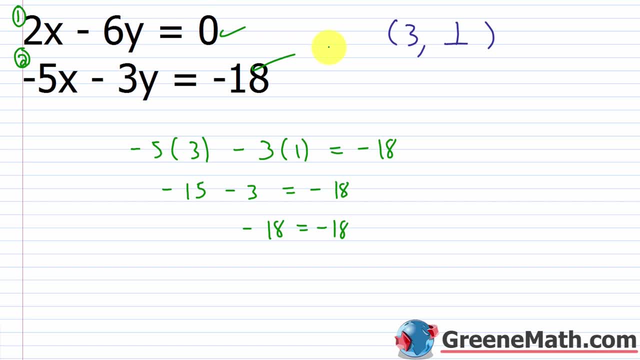 Or again, an x value of 3, a y value of 1.. All right, let's take a look at another example. So we have negative: 3 equals 3y plus 3x. We have 7 fourths. y equals x plus 15 fourths. 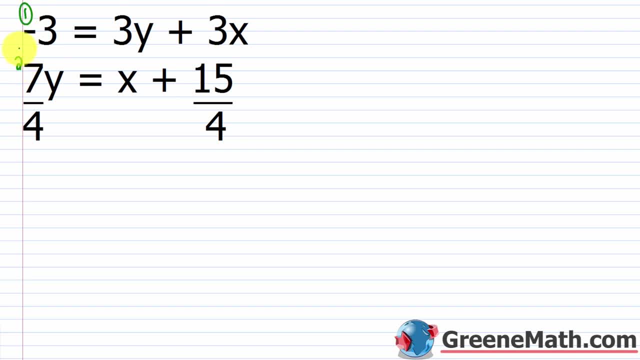 So this is equation 1, and this is going to be my equation 2.. If I want it to look like this: ax plus by equals c. So for my first equation I could just simply write it as 3x plus 3y. 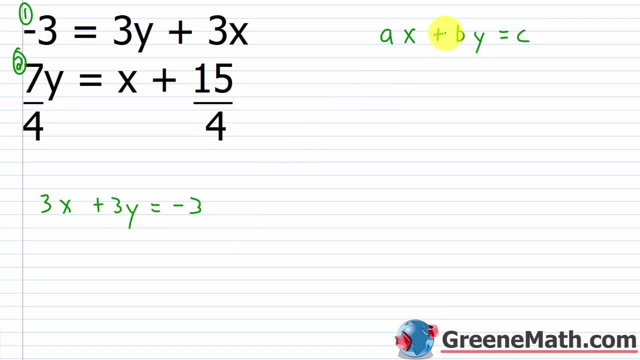 is equal to negative 3.. So that solves that. For the second equation, I can subtract x away from each side. So let me write this over here: If I have 7 fourths, y is equal to x plus 15 fourths. 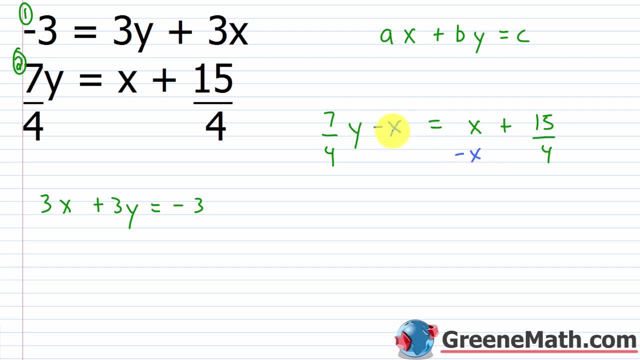 I can subtract x away from each side of the equation. That'll cancel. So I can reorder this and just put negative x out in front. plus 7 fourths, Y is equal to 15 fourths. Now it's not necessary to do this. 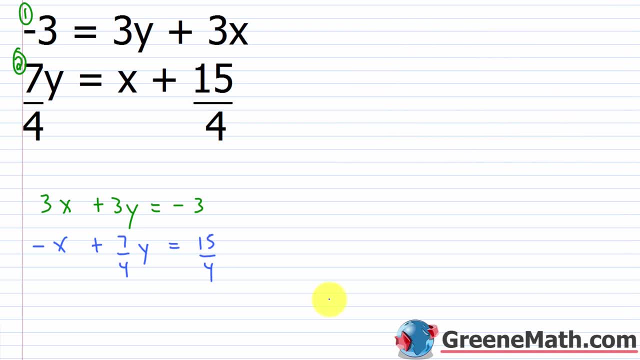 but it's more convenient to work with equations that don't have fractions. So go ahead and do yourself a favor. Multiply both sides in this equation by 4 and get rid of those denominators. So 4 times negative x is negative 4x. 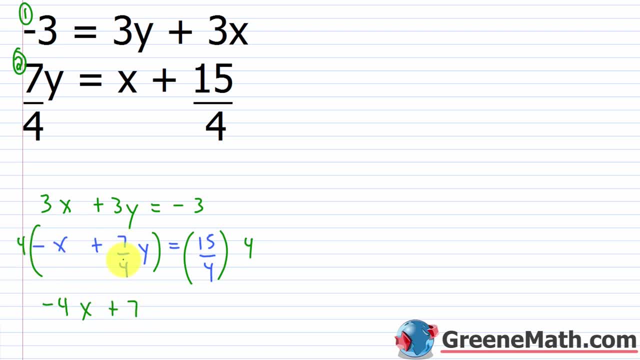 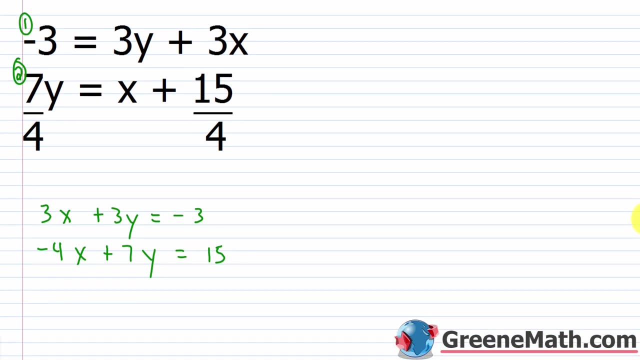 4 times 7, fourths is 7.. So this would be plus 7y. This equals 4 times 15, fourths is 15.. So let's erase all of this and we'll drag this up here. OK, let me scroll down and get a little room going. 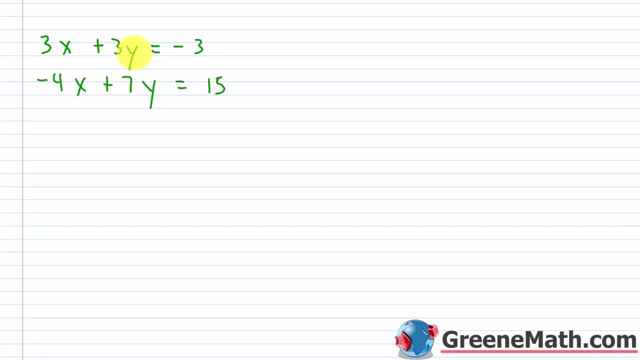 Now what we see is we have 3x and negative 4x, 3y and 7y, But what would be easier to make into opposites? Well, both of them would be about the same amount of work, And what I can do is I'll just go with our target x. 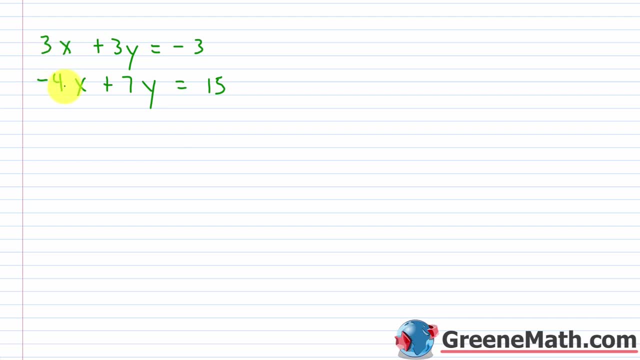 So the target x, we think about 3 and negative 4.. The least common multiple between the two would be 12.. So I want one to be positive 12 and one to be negative 12.. Well, that's really easy to do. 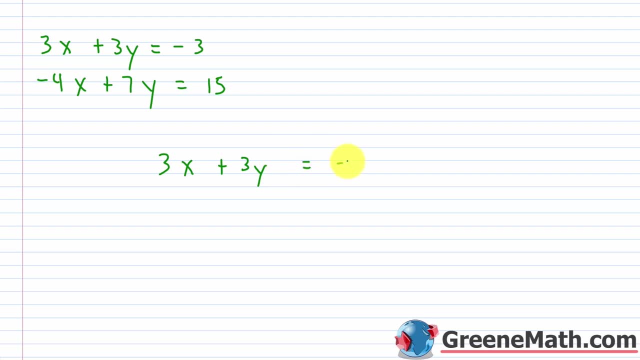 If I have 3x plus 3y equals negative 3, I can multiply both sides of this equation by positive 4.. And what that is going to give me: 4 times 3x is 12x. 4 times 3y is plus 12y. 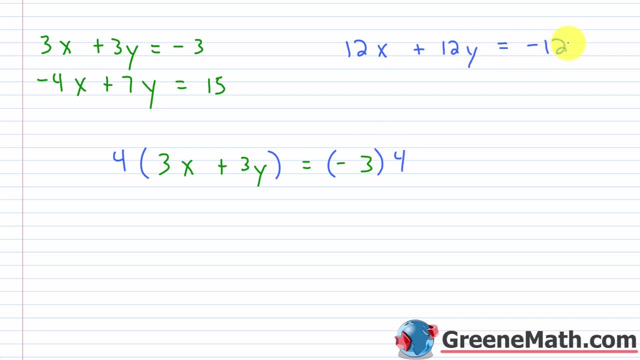 This would be equal to 4 times negative 3, plus negative 12.. Let's erase that Then for this one, if I have negative 4x plus 7y equals 15.. Again, I want negative 12 here. 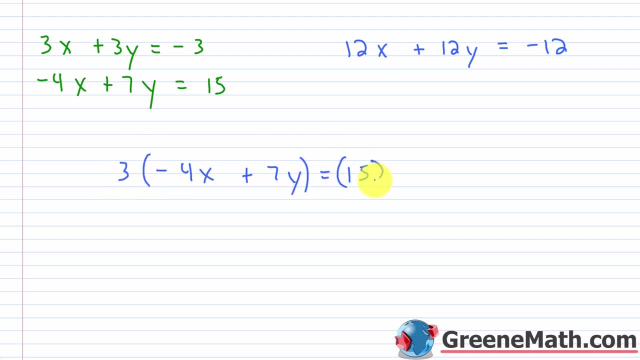 So I would multiply both sides of this equation by 3.. So 3 times negative 4x is negative, 12x. 3 times 7y is 21y, And then 3 times 15 is 45. So now I have a pair of variable terms that are opposites. 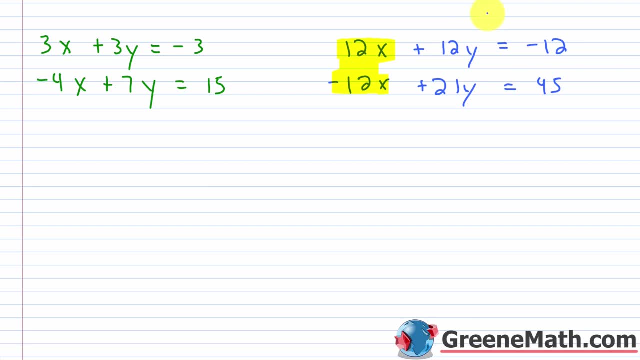 I have 12x and negative 12x, So we're basically good to go. We would add the left sides together. We'd set this equal to the sum of the right sides. So 12x minus 12x, that's 0x, or just 0.. 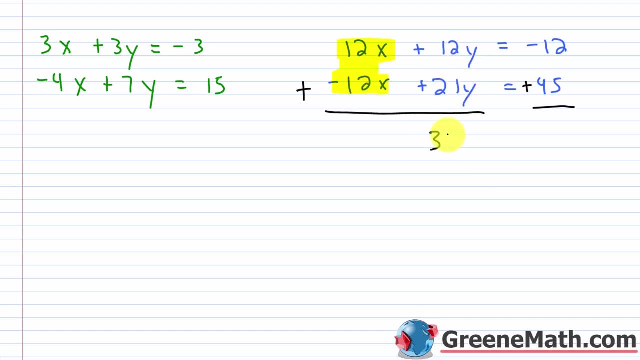 12y plus 21y would be 33y And this equals negative. 12 plus 45 is 33.. So if I divide both sides, if I divide both sides of the equation by 33, I would get that y is equal to 1.. 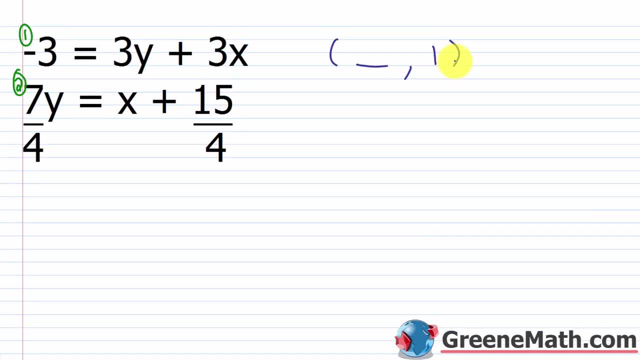 So our ordered pair would be something for x, 1 for y. Now I can plug a 1 in for y in either equation 1 or 2.. Looks like it's a whole lot easier to work with equation 1, because again I'll have to deal with those fractions. 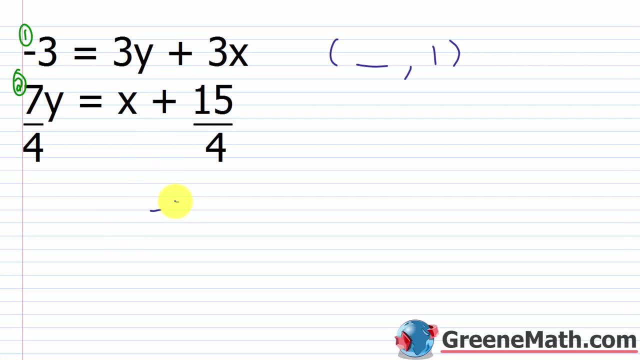 So let's go ahead and do negative 3.. Negative 3 is equal to 3 times y. y is 1, so 3 times 1, plus 3x. So I'd have negative: 3 is equal to. this will just be 3, plus 3x. 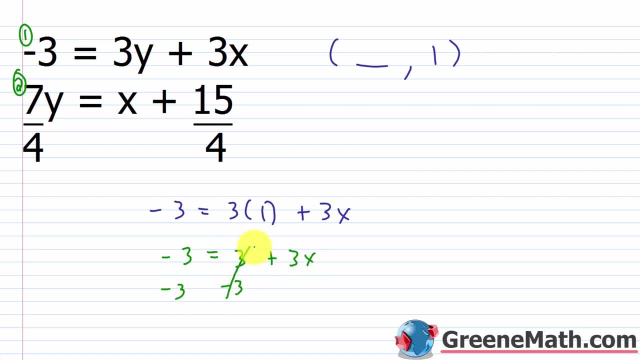 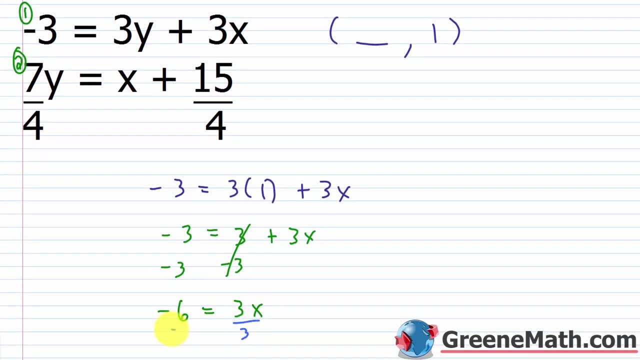 Let's subtract 3 away from each side of the equation. That'll cancel. I'll have negative 6 is equal to 3x. Let's now divide both sides by 3. And what I'll have is x is equal to negative 2.. 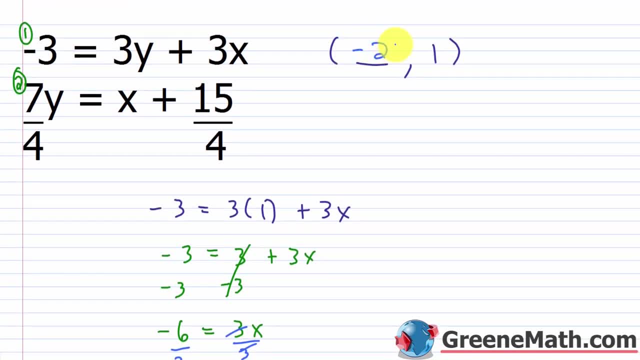 So x here is negative, 2, y is 1.. All right, so let's go ahead and plug in to each original equation We have: negative 3 is equal to 3 times y, y is 1, plus 3 times x. 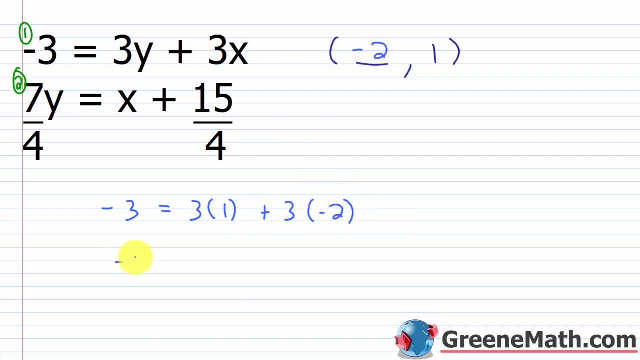 x is negative 2.. So I'd have negative 3 is equal to. we know 3 times 1 is 3.. 3 times negative 2 is negative 6.. So if I had 3 plus negative 6, that would be negative 3.. 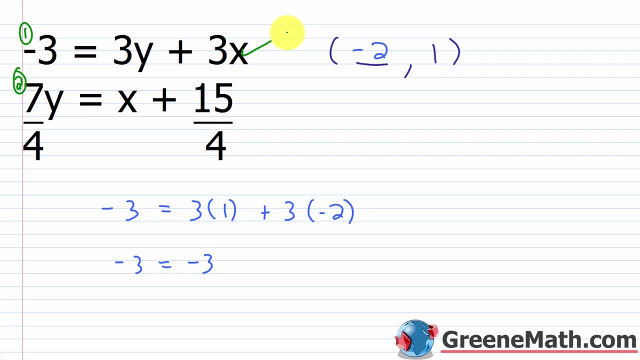 So you get negative 3 equals negative 3.. So it works out here. For the next one, I have 7 fourths times y. y is 1. This equals x, which is negative 2, plus 15 fourths. 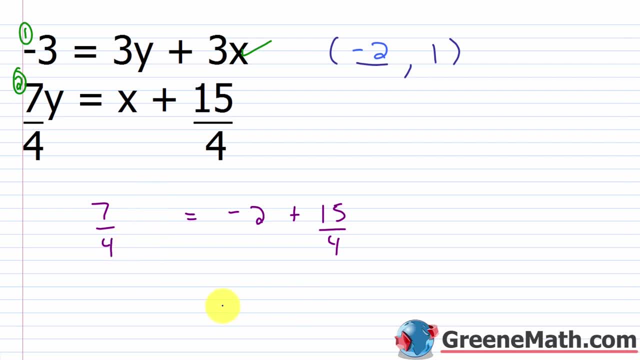 So we know 7 fourths times 1 is just 7 fourths, So just you can erase that. For this one I need a common denominator, So I'll multiply this by 4 over 4.. So I'd have negative 2 times 4, that's negative 8.. 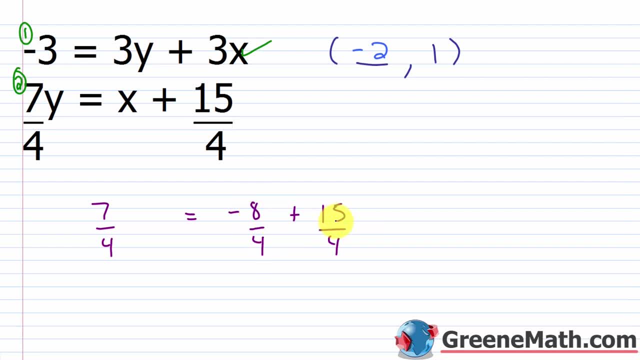 Negative 8 over 4.. Now if I had negative 8 and 15, I get 7 over the common denominator of 4.. So yeah, this is going to be: 7 fourths is equal to 7 fourths, So it works out here as well. 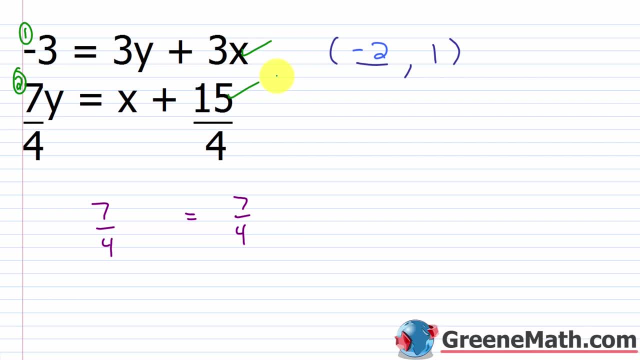 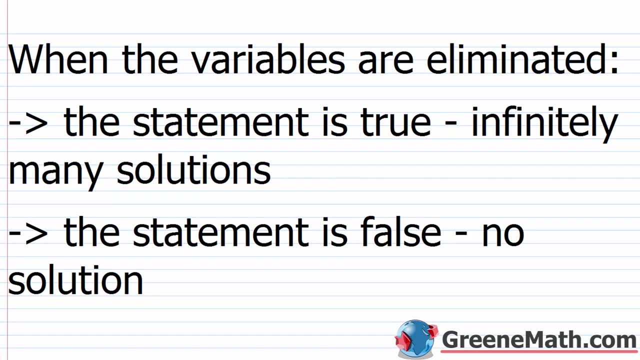 So our ordered pair negative 2 comma 1, or an x value of negative 2 and a y value of 1, is our solution for the system. Now we've already seen this in the substitution video When the variables are eliminated. 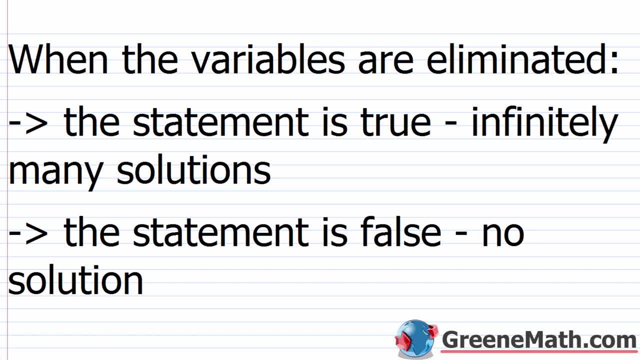 all of them, there's nothing left in the equation you're working with. when the statement is true, there's infinitely many solutions. So if you get something like 15 equals 15,, 29 equals 29,, 35 equals 35, you know, so on and so forth. 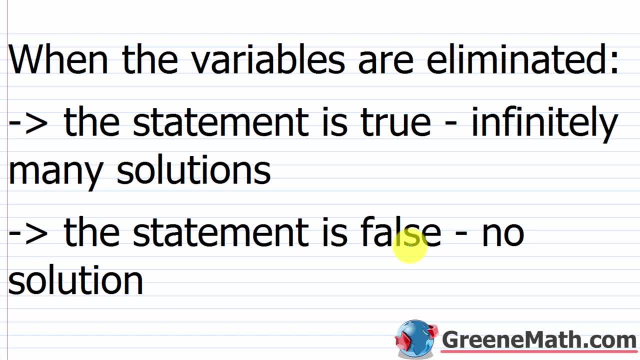 If the statement is false, so 3 equals negative 2, 7 equals negative 21,. you know, so on and so forth. there's no solution. So in this case, right here. the second case: there are parallel lines. 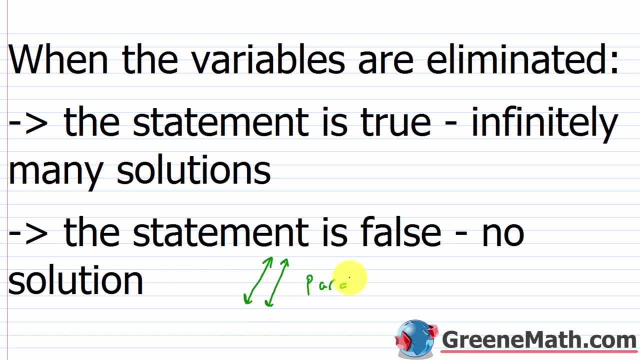 So there are parallel lines. In this case it's the same line. It's the same line, It's just algebraically manipulated to look different. And the way you can tell for sure for this type, where there's an infinite number of solutions. 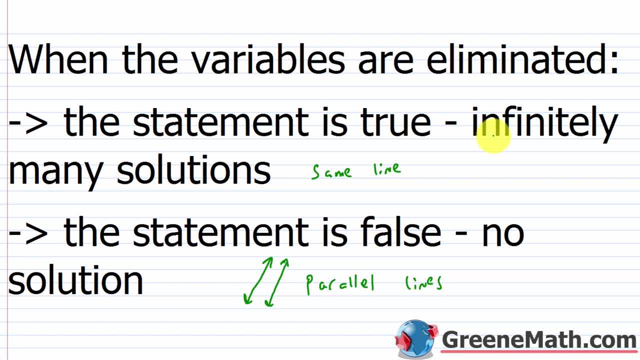 just solve the equations for y. you're going to see you have the same equation For this one where there's no solution. solve the equations for y. you're going to see you have the same slope but different y intercepts. so you know you have parallel lines. 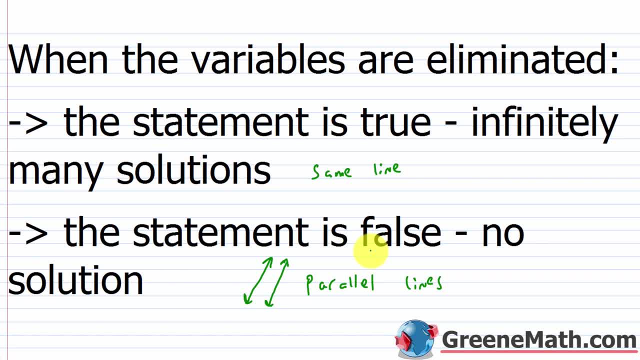 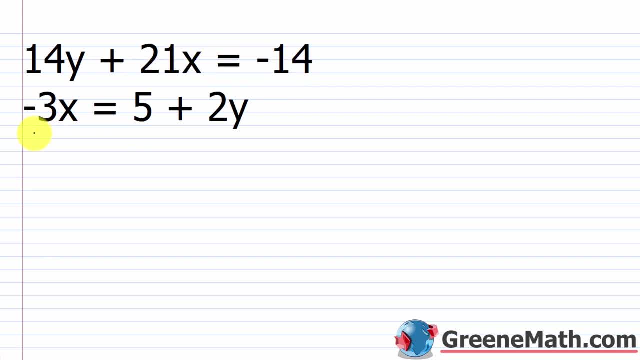 Parallel lines don't intersect, so there's no possible solution. Alright, let's take a look at some special case scenarios. So you have 14y plus 21x equals negative 14.. You have negative 3x equals 5 plus 2y. 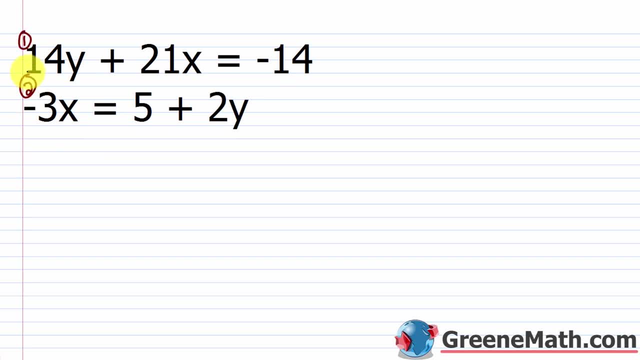 So let's say this is equation 1,, this is equation 2.. So for equation 1, again, we want to put this in ax plus by equals c or standard form, And so all I'm going to do is just switch the order. 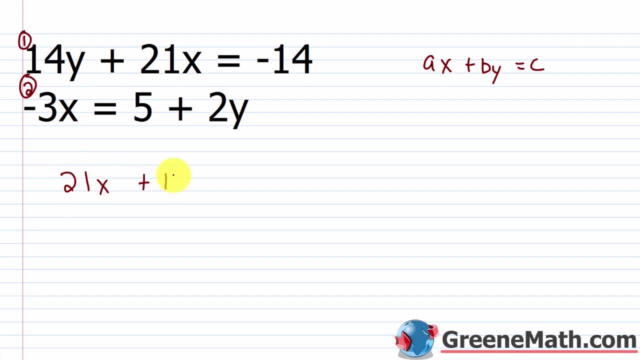 So I would write this as: 21x plus 14y is equal to negative 14.. For this one, if I have negative 3x, negative 3x is equal to 5 plus 2y. all I need to do is subtract 2y away from each side of the equation. 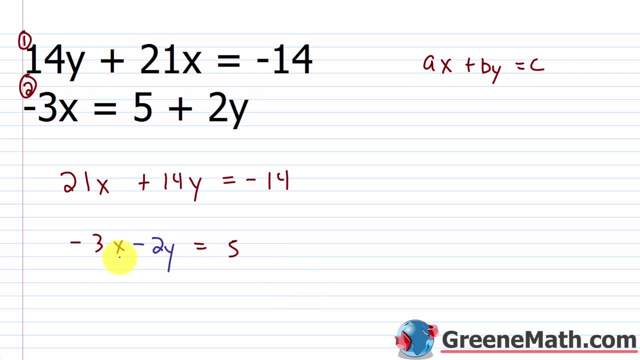 So this would cancel. So I'd have: negative 3x minus 2y equals 5.. So let me kind of write that a little better: Negative 3x minus 2y is equal to 5.. Alright, so now I'm looking to make one pair of variables. 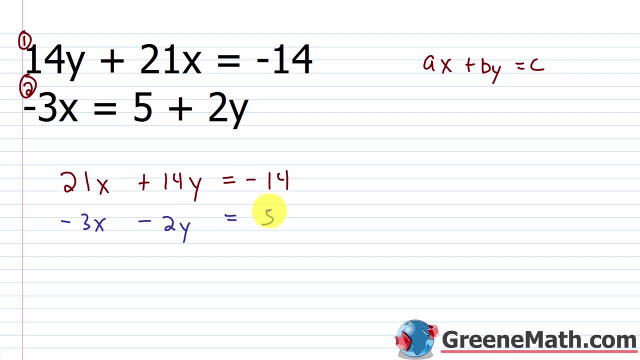 into one pair of variable terms, into opposites, And again you can pick either one. here It's about the same amount of work. You have negative 3 and you have 21.. So obviously, if I multiply negative 3 by 7, I would get negative 21 there. 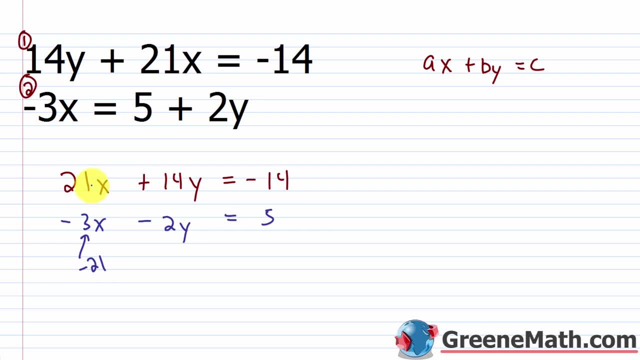 So the coefficient here would be negative 21.. The coefficient here would be positive 21.. Equally as easy, if I multiply this guy here by positive 7, negative 2 times positive 7 would be negative 14.. Negative 14 and positive 14 are opposites. 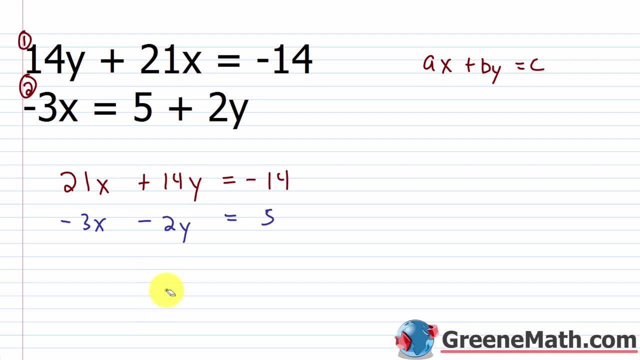 Whatever you want to do, I'm just going to go with x, because that's the first one. So if I multiply both sides of this equation by 7, then what I'd have is negative 21x minus 14y is equal to 35.. 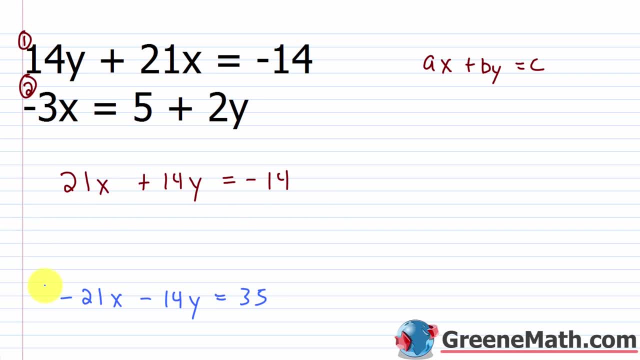 So I can just erase this one and I'll drag this up And now we can add the left sides together. set that equal to the sum of the right sides. So plus, plus. Now you can see right away: 21x minus 21x is 0.. 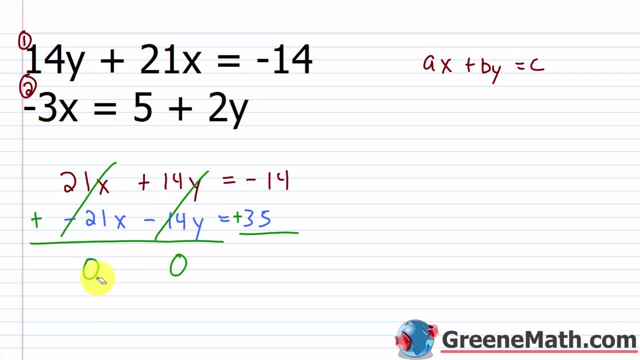 14y minus 14y is 0. So I would have 0 on the left And this equals negative. 14 plus 35 is going to give me 21.. So is this a nonsensical statement? 0 equals 21.. 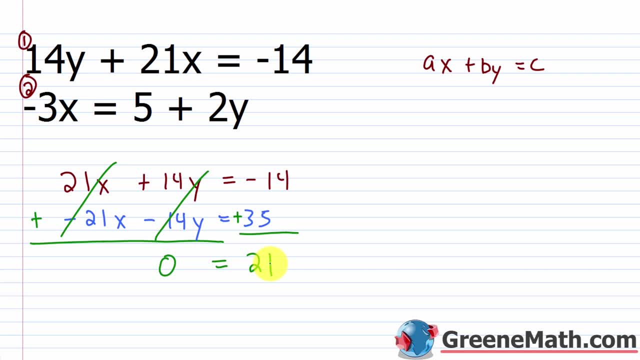 Yes, it is. It's obviously not true. So this is the case where we have two parallel lines. So there's no solution. So there's going to be no solution. And if you want to prove this to yourself, go ahead and pause the video. 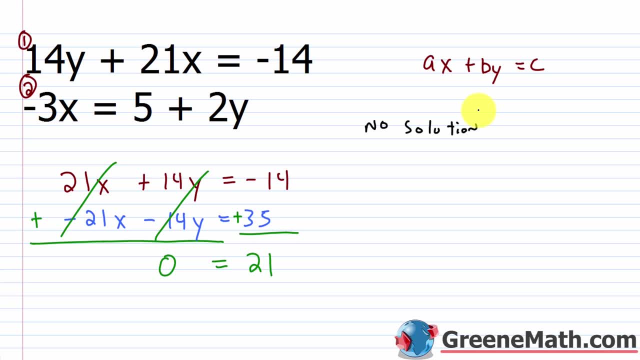 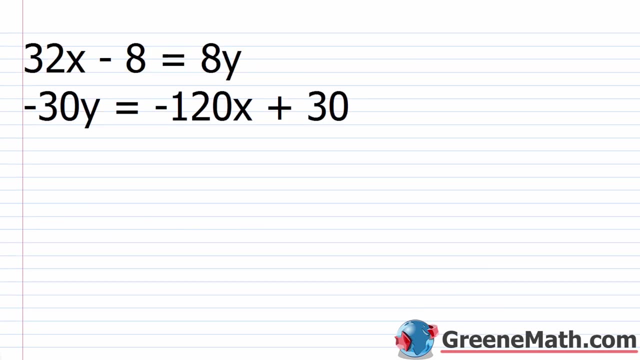 Solve each equation for y, You're going to find that you have the same slope and different y intercepts in each case, So they're parallel lines. We can also do this and we can say they're parallel lines. Let's take a look at another example. 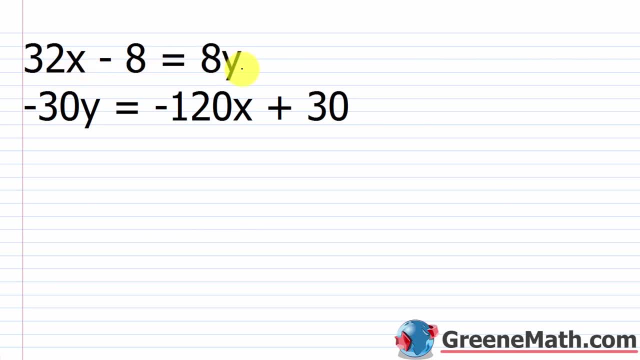 So suppose we see 32x minus 8 equals 8y Negative. 30y equals negative 120x plus 30. So again I want this in standard form. So ax plus by equals c. So for this guy again I'm going to label these equations. 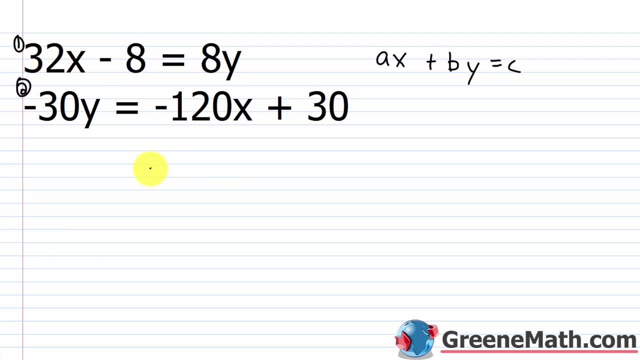 Equation 1 and equation 2.. For equation 1, if I have 32x minus 8 equals 8y. Let me add 8 to each side of the equation. Let me subtract 8y from both sides of the equation. 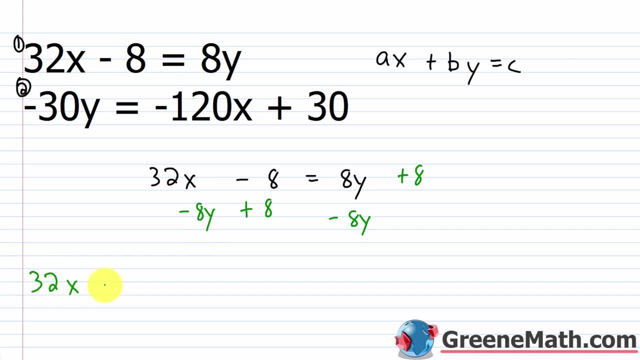 So that's going to give me 32x minus 8y is equal to positive 8.. Then for equation 2, all I need to do is add 120x to each side of the equation I will have: 120x minus 30y is equal to 30. 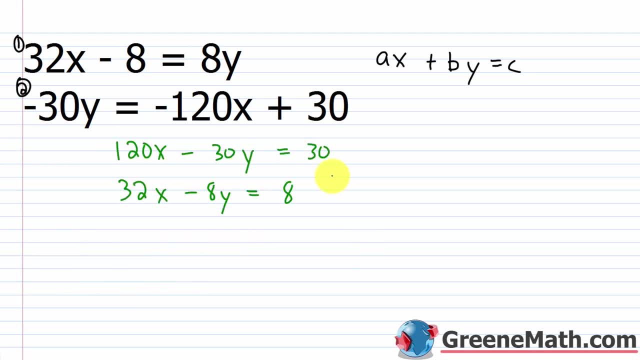 All right. So this one's a little more tedious And I would just choose the smaller coefficients here. So I'm going to work with y. So if I have negative 30 and I have negative 8.. Forget about the signs for a second. 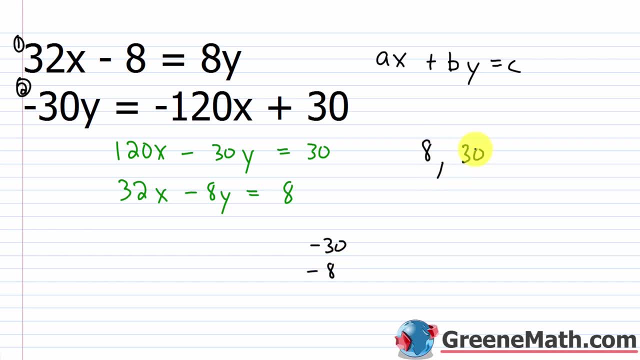 Just pretend you have 8 and you have 30.. What's the least common multiple there? What's the least common multiple? Well, 8 is what It's 2 times 2 times 2.. 30 is what It's 6 times 5.. 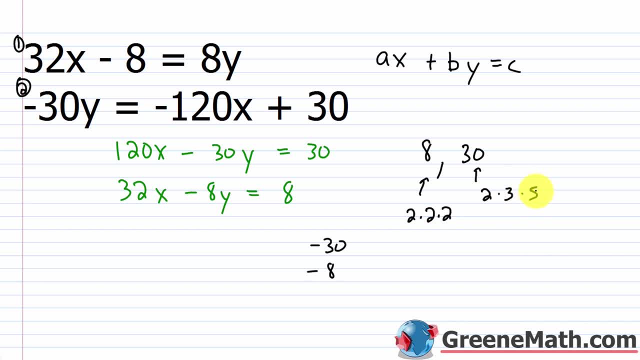 Or it's 2 times 3 times 2.. It's 3 times 5.. So really it would be 2 times 2 times 2 times 3 times 5.. Or 8 times 15, which is 120.. 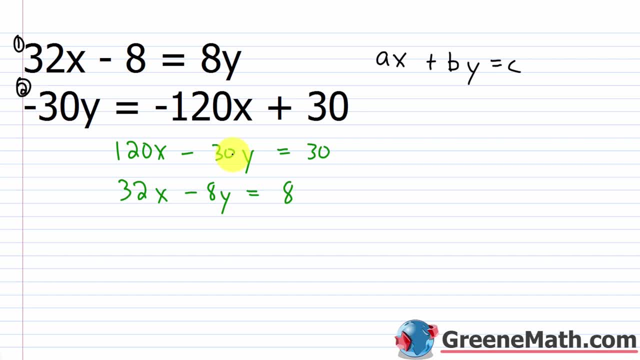 So if I think about 120, I want one of these to be negative 120y, the other to be positive 120y. So let me multiply both sides of this equation by a negative 15.. Now let me multiply both sides of this equation. 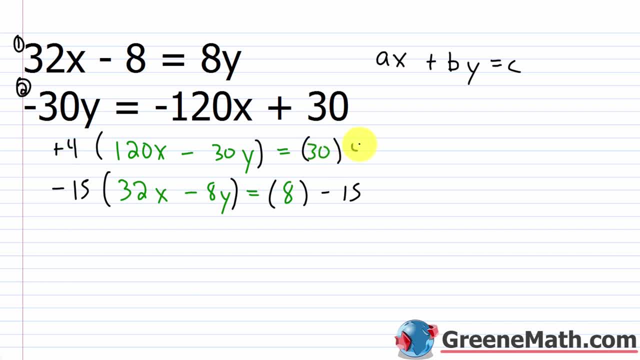 by a positive 4.. So 4 times 120x is 480x. 4 times negative 30y is minus 120y. 4 times 30 is 120.. For this guy, negative 15 times 32 is negative 480.. 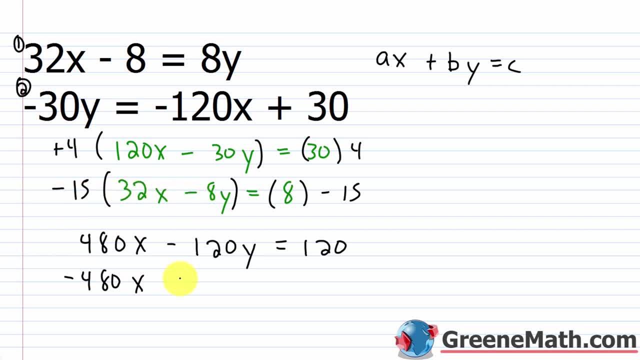 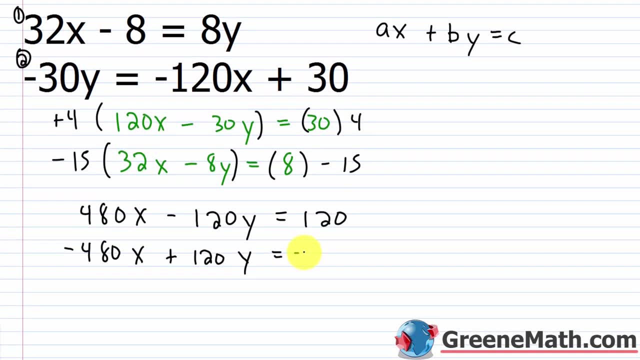 Then of course, times x- Negative 15- times negative 8 is positive 120.. Then times y Equals 8 times negative 15, which is negative 120.. So if I want to add the two left sides here together and I want to add the two right sides here together, 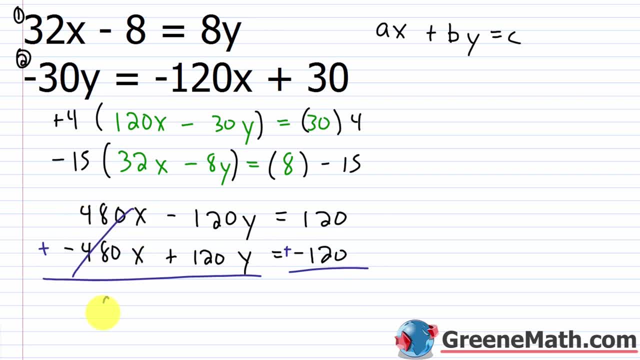 480x minus 480x is 0. Negative. 120y plus 120y is 0.. 120 minus 120 is 0.. So what do I get? I get 0 equals 0, which is true. So the variables have dropped out. 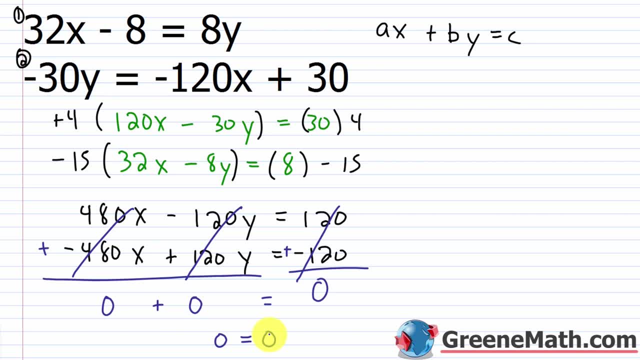 and I'm left with a true statement. So there's an infinite number of solutions. Right, These two equations are basically the same. They've just been algebraically manipulated to look different. So there's an infinite number of solutions. And again, you can solve each equation for y. 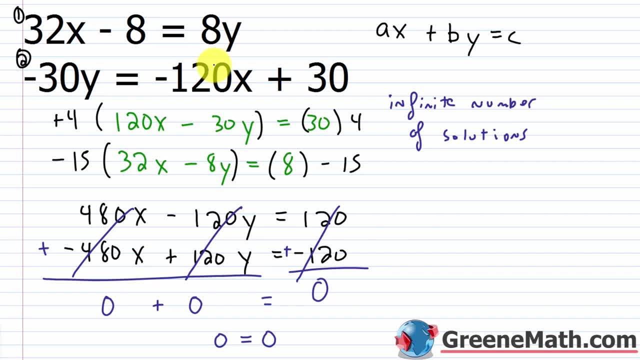 That'd be the easiest thing you can do, And if you solve each equation for y, you're going to see that you have the exact same equation in each case And therefore, whatever works in equation 1 also works in equation 2, because it's the same equation. 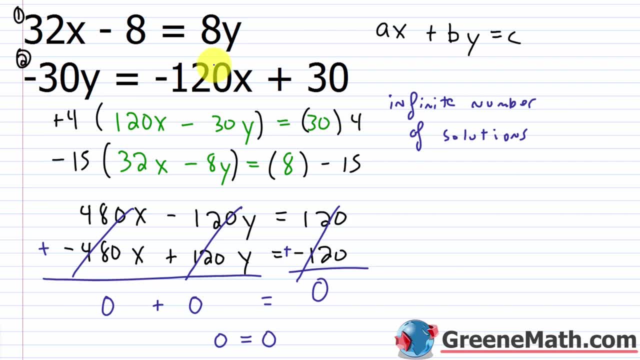 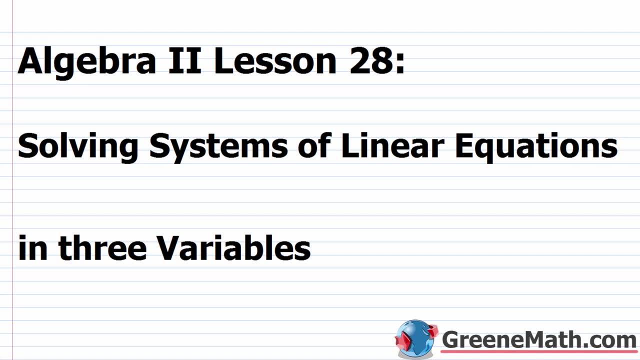 So there would be an infinite number of solutions for this system. Hello and welcome to Algebra 2, Lesson 28.. In this video, we're going to learn about solving systems of linear equations in three variables. So up to this point, we've become very familiar. 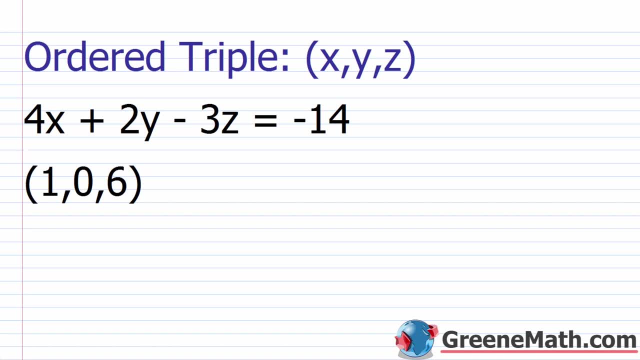 with how to solve a system of linear equations in two variables, using graphing, using substitution and using elimination. Now we're going to rely on all this knowledge to get us through the next challenge, which is solving a system of linear equations in three variables. 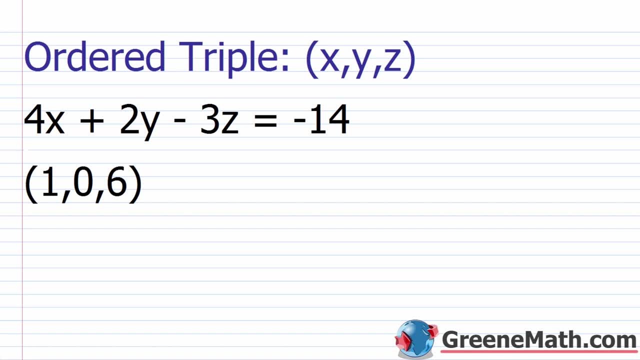 Before we learn how to solve that type of system, we first need to familiarize ourselves with a linear equation in three variables. So a linear equation in three variables looks like this: It's ax by plus cz equals k, So just something times x plus something times y. 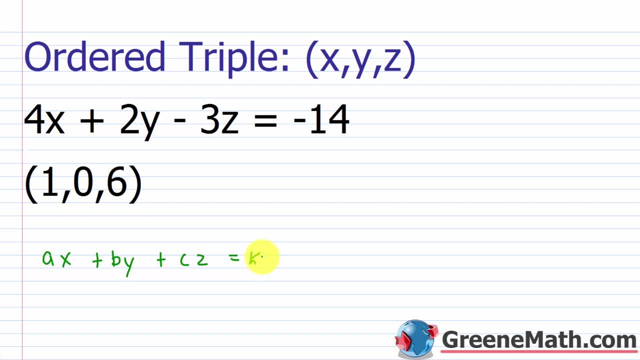 plus something times z equals some constant. So we would say: a, b, c and k are just real numbers, where a, b and c are not all zero at the same time. Because again, if you had that, your variables would all drop out. 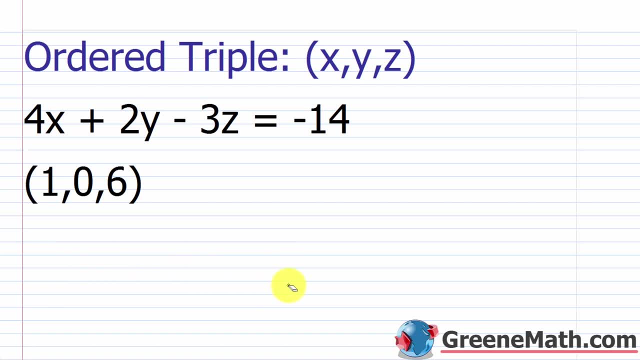 Alright, so let's look at an example of this real quick. I think if we just use our prior knowledge of working with a linear equation in two variables and extend it to a linear equation in three variables, we're pretty much good to go. 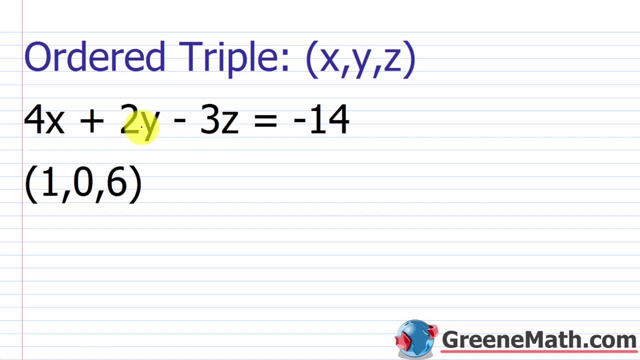 We've just added a variable here. So we have 4x plus 2y minus 3z equals negative 14. And I have a sample solution. okay, We know, when we work with a linear equation in two variables, we give our solution as an ordered pair. 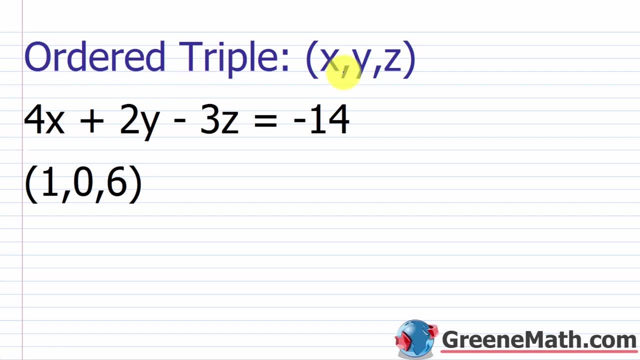 Now we're going to have a solution as an ordered triple. So instead of just an xy, it's an x, a, y and a z, And it's in that order. So, as this example goes, I have this order triple. 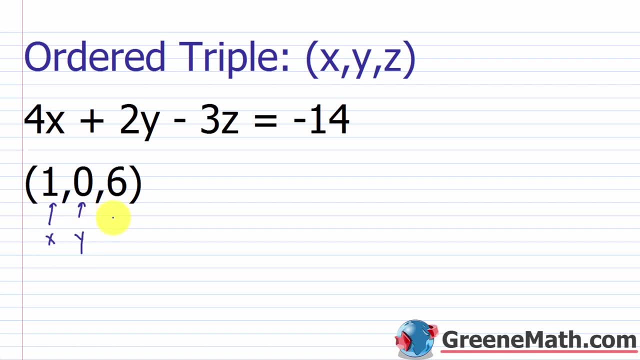 This 1 is an x, this 0 is a y and this 6 is a z. So I should be able to plug in a 1 for x, a 0 for y and a 6 for z, and I should get a true statement. 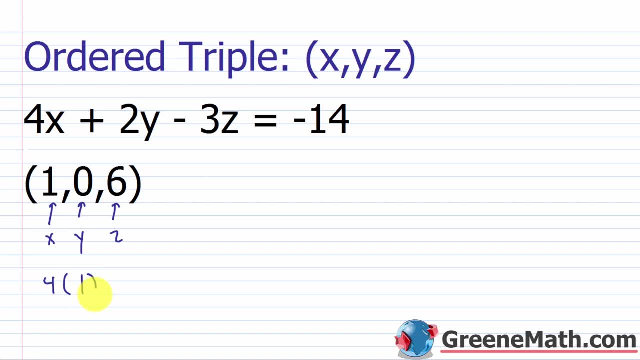 So I would have 4 times 1,. plug in a 1 for x plus 2 times 0,. plug in a 0 for y minus 3 times 6, plug in a 6 for z, And this should equal. 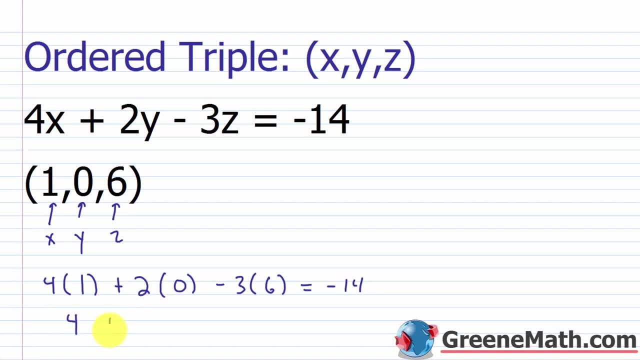 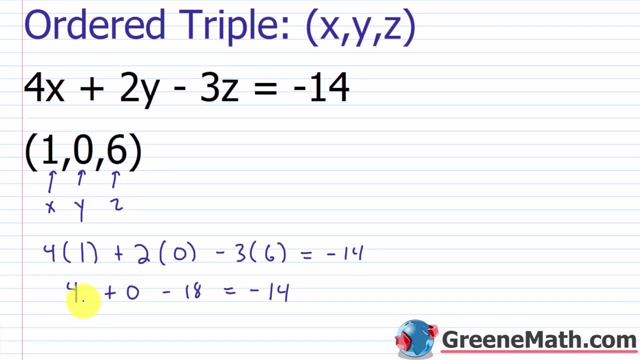 negative 14.. So 4 times 1 is 4,, 2 times 0 is 0, negative. 3 times 6 is negative 18.. This should equal negative 14, and it does. You basically have 4 minus 18,, which is negative 14.. 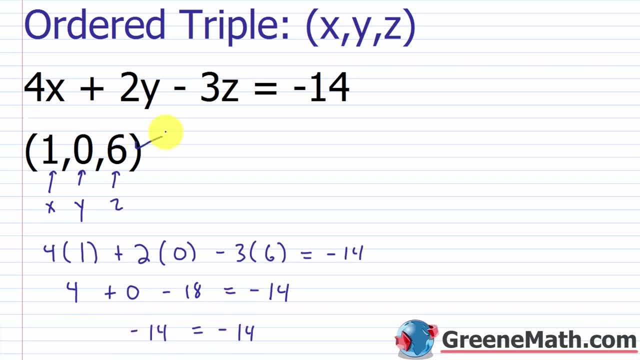 So that does equal negative 14.. So this works as a solution. But just like we saw with a linear equation in two variables, a linear equation in three variables is also going to have an infinite number of solutions. So I could just generate as many, ordered. 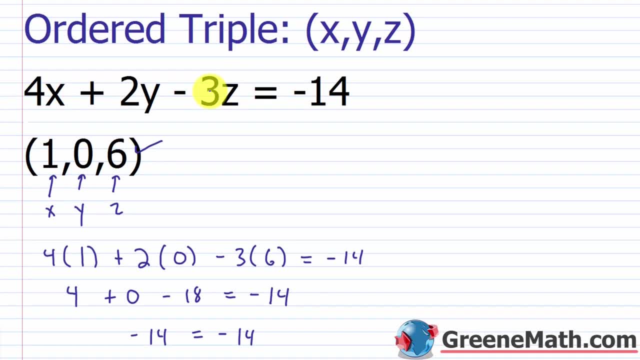 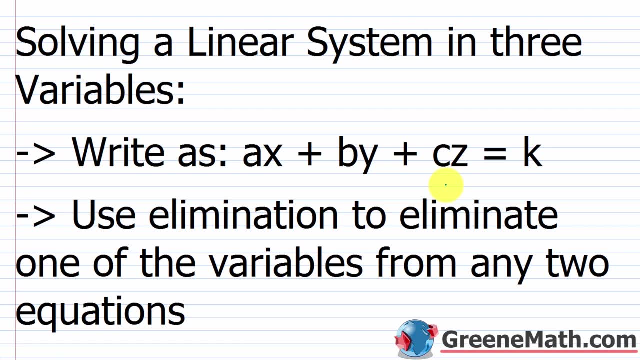 triples, as I want as solutions for this equation. All right, So now that we know what a linear equation in three variables is, what if we get a linear system in three variables? So this is going to contain three equations with three unknowns. 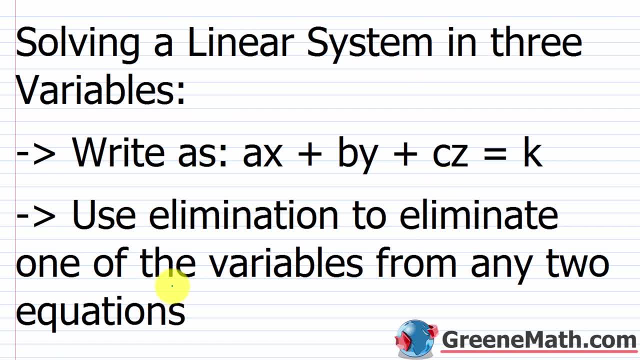 So solving a linear system in three variables, The first thing we want to do is we want to write each as ax plus by plus cz equals k. Why do we do this? Well, we're doing it because we're going to do some elimination with elimination. 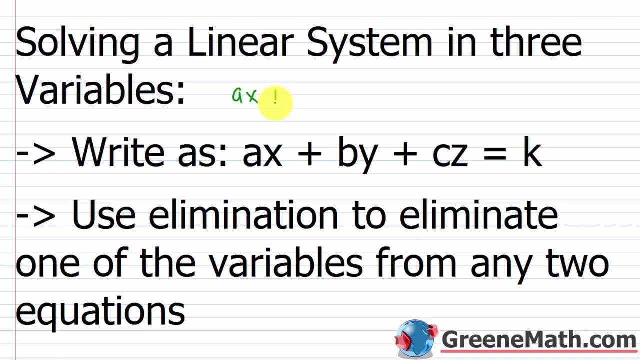 We remember, our first step is to write ax plus by equals c when we have two variables involved. Well, it extends to this. with three variables, I just have plus cz. The reason we do this is because we make it easy to see what we're going to be able. 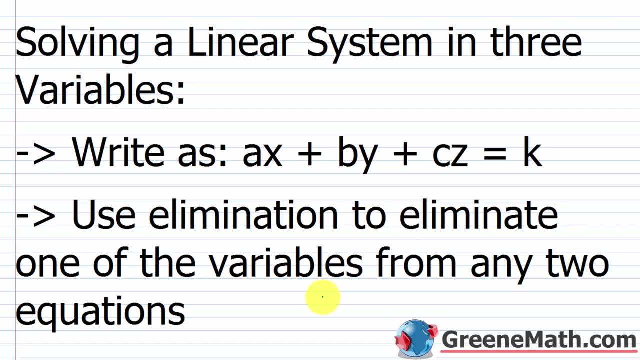 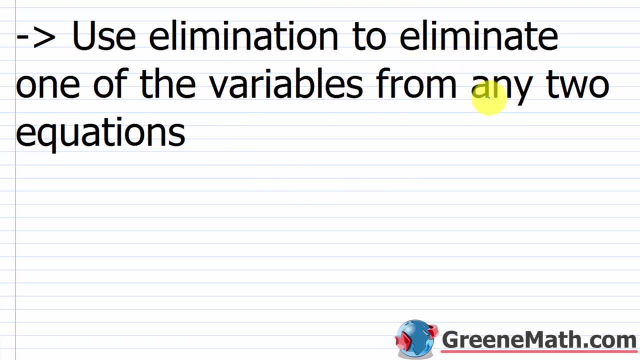 to eliminate, or what we would need to eliminate a variable. All right, So now that we've done that, we use elimination to eliminate one of the variables from any two equations. It doesn't matter what variable you pick. It doesn't matter what two equations you pick. 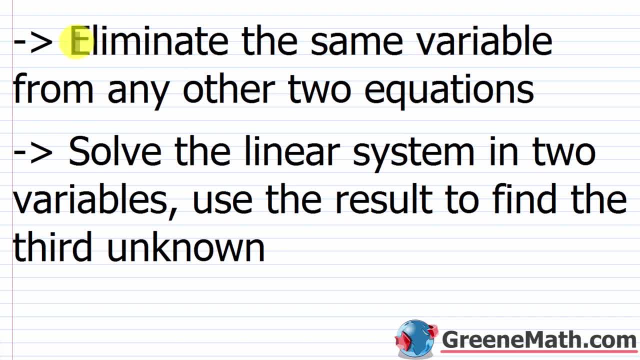 But in the next step it does matter. You need to eliminate the same variable from any other two equations. So if in that last step I eliminated x, when I get to this step I've got to eliminate x again. What that's going to do is it's going to give me a linear system in two variables. 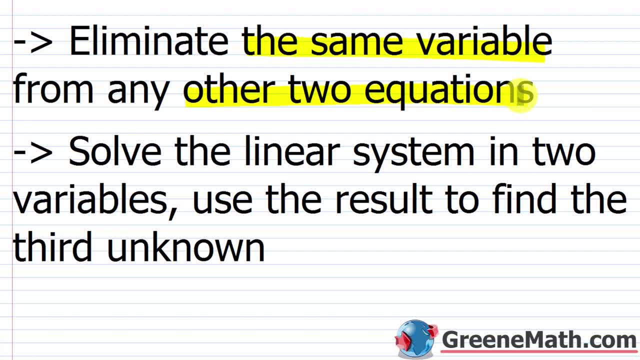 If I eliminated x, I have y and z. Once I have a linear system in two variables. we already know how to solve that. So solve the linear system in two variables. You can use substitution or elimination, whatever you want to do. 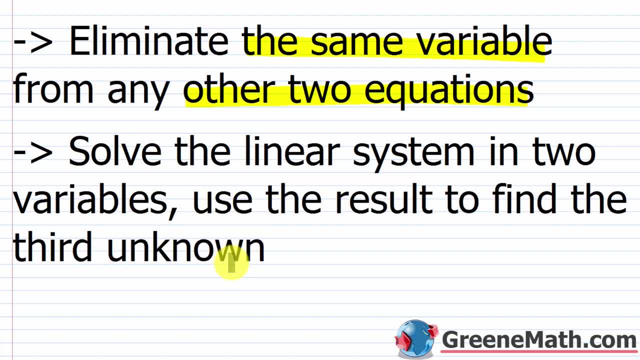 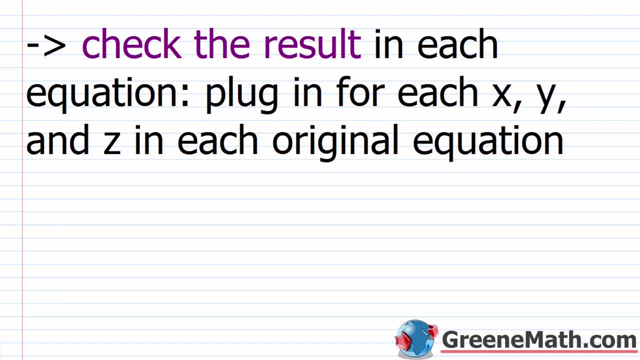 Use the result to find the third unknown. Once I know what two of them are, I can go back to any original equation and find the third unknown. The last step, and always the most important, check the result in each equation. So you're going to plug in for each x, y and z in each original equation. 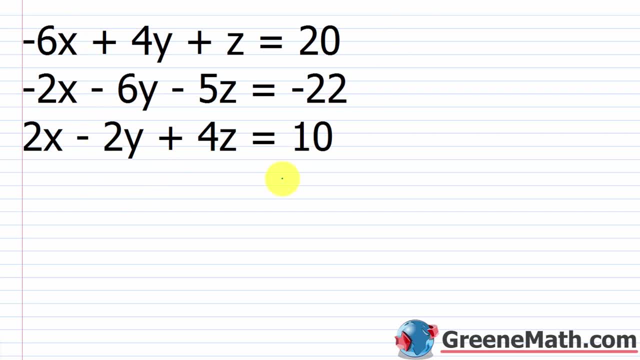 Now the one thing that always comes up and a lot of students ask this. they say: can you use substitution the whole way through? So, in other words, can I use substitution to generate a linear system in two variables and then solve that with substitution and end up with the answer? 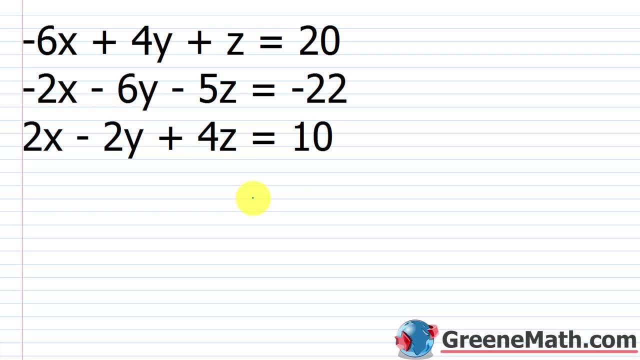 for my linear system in three variables. The answer to that is yes, you can do that. The reason that we generally don't teach that is because it's super tedious If I solve one of these or one of the variables and then I plug that in to the 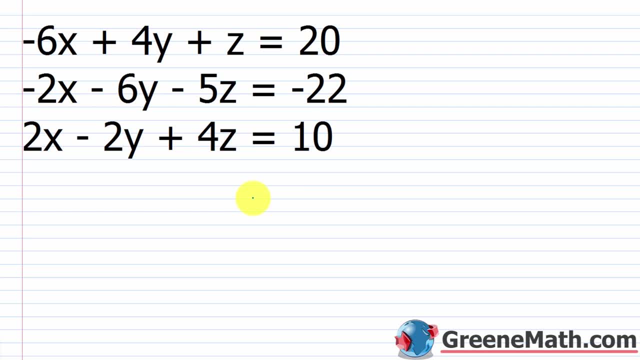 next two equations, I will generate a linear system in only two variables, But to do it will be super, super tedious And it's very prone to errors because of that. So let's start out with what we have. We have negative six. x plus four. y plus z equals 20.. 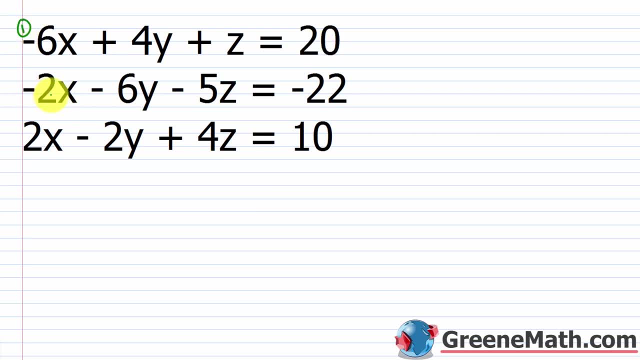 I'm going to call this equation one. Then I have negative two x minus six, Y minus five, z equals negative twenty two. I'm going to call this equation two. And I have two x minus two, y plus four, z equals ten. I'm going to call this equation three. 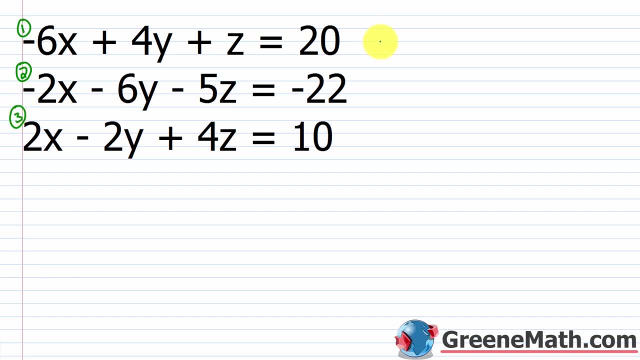 Now everything is already written for us, as we were told to do, as a, x plus b, y plus c, z equals k, So we don't need to do anything on that front. We move immediately into picking one variable to eliminate between two equations. So if you look at everything, 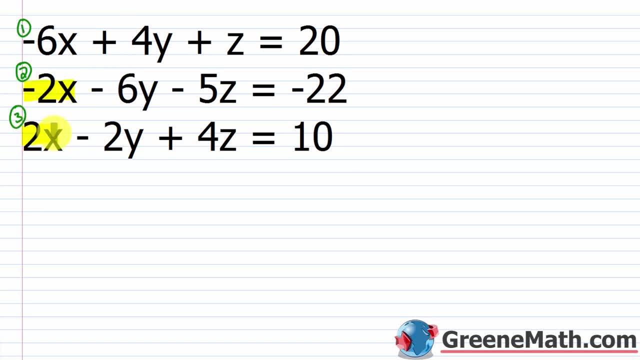 it looks like it's pretty easy to eliminate x between equation two and three. I've got negative two x and I've got two x, So that would work out pretty nicely for us. So if I've got negative two x minus six, y minus five, z equals negative twenty two. 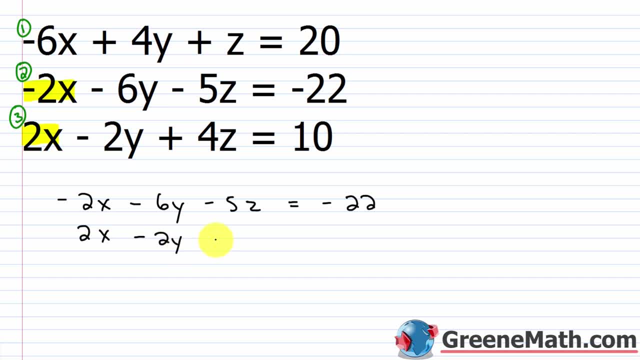 And if I've got two x minus two y plus four z equals ten. I can sum the left side, I can sum the right sides together and set this equal to the sum of the right sides. So negative two x plus two x is zero. 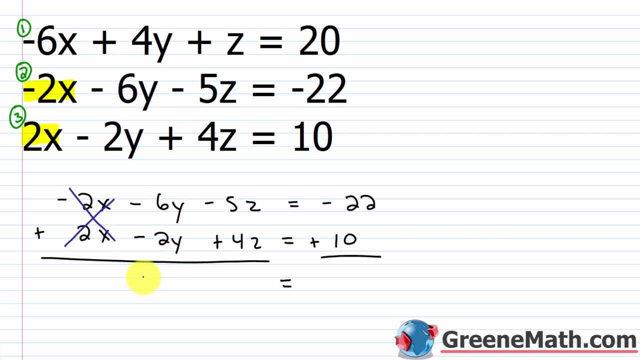 X has been eliminated. Negative six: y minus two. y is negative eight y. Negative five: z plus four. z is negative z And negative twenty two plus ten is negative twelve. So I've produced an equation that is x free. So let's call this equation four. 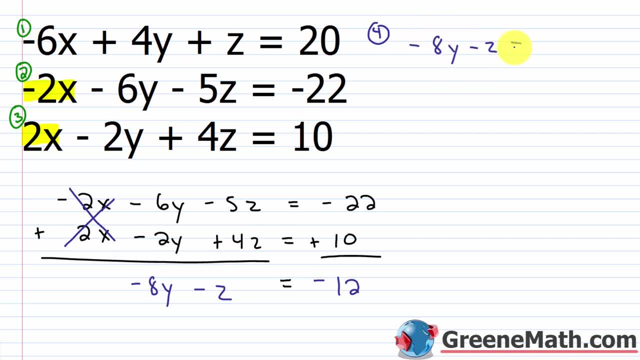 This is negative eight y minus z, So I've got negative six y minus two y plus four z equals negative twelve. Right now, the next thing I want to do is I want to get any other two equations, So I worked with two and three. 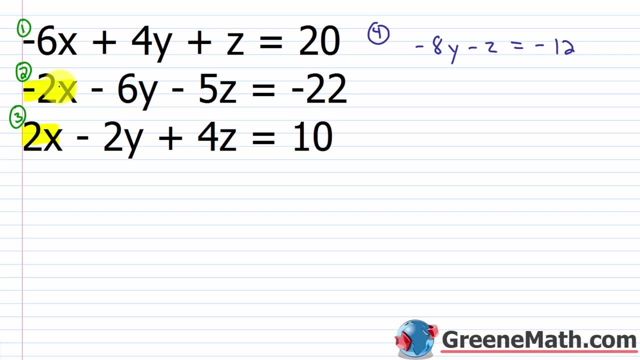 So it either needs to be one in three or one in two. So one of those scenarios, I need to eliminate x from those. So let's go ahead and just do one in three, because I have a negative six and a positive two, So the coefficients are opposite signs. 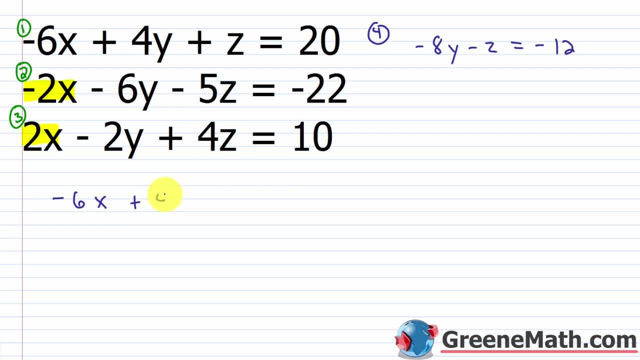 It's a little bit easier. So we have negative six x plus four, y plus z equals twenty. And then for equation three, I have two x minus two, y plus four, z equals ten. Now if I want to make these opposites, I can multiply two x by three. 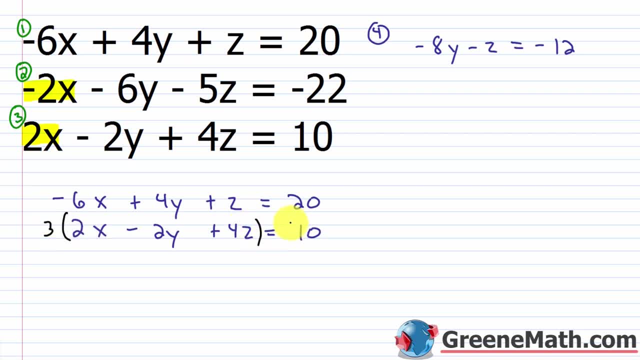 But to make that legal I've got to multiply both sides of the equation by three. So three times two x is six x. Three times negative two y is negative six y. Three times four z is plus twelve. z Three times ten is thirty. 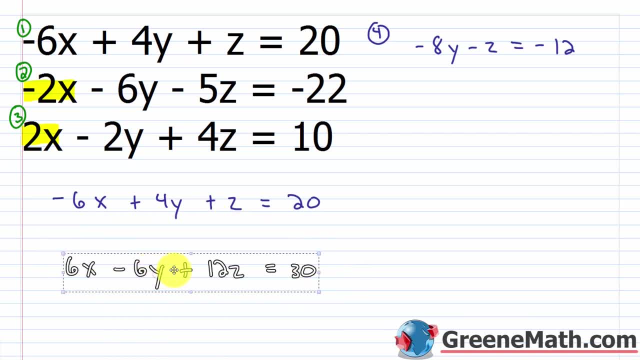 All right, so let's erase this and we'll just drag this up here And again. I'm going to add the two left sides. Set this equal to the sum of the right sides. Negative six x plus six x is zero. So again, x has been eliminated. 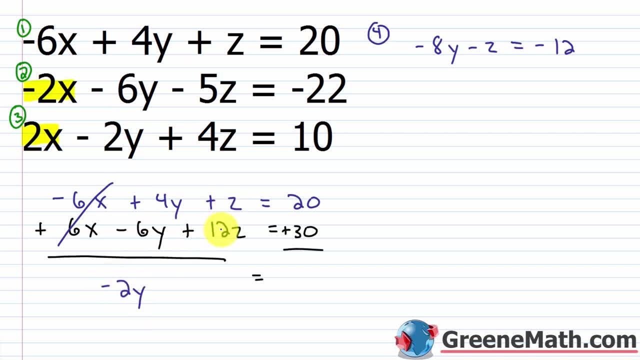 Four y minus six y is negative. two y Z plus twelve, z is plus thirteen z. Twenty plus thirty is fifty. So what this would produce? let me kind of move this down. be in line For equation five. we'll call it. 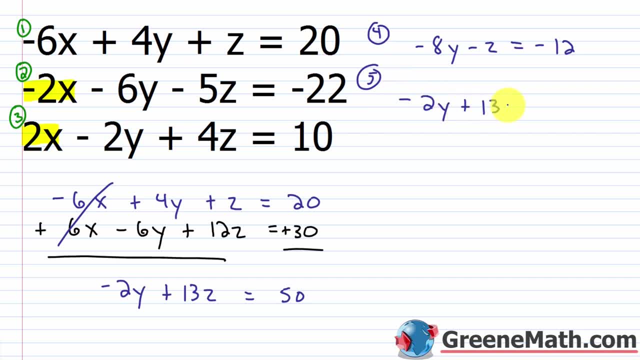 This would be negative. two y plus thirteen z equals fifty. Now let me erase this. I have produced a linear system in two variables, So now we know how to solve this. We've been doing this forever now. The only other side note I would say is we did that so much quicker than if I, let's say, solved for z. 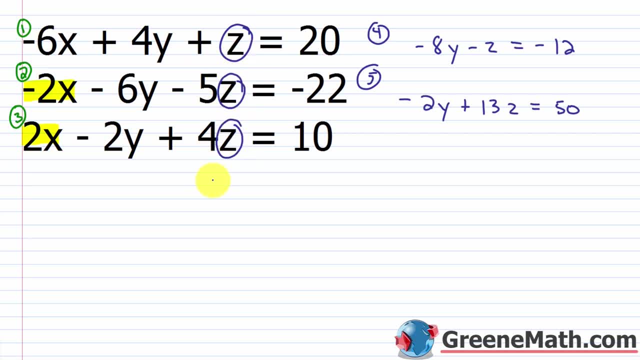 And then I plugged in for z in this equation and this equation Again, that's the substitution method you could use. That would produce a linear system in two variables with just x and y, And then I could, I could solve that as well. 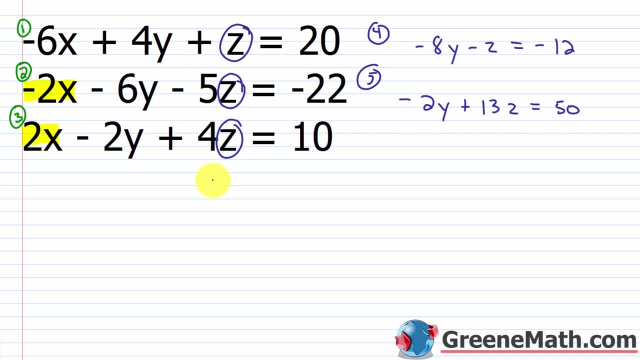 But again, using that method is just ultra tedious And I want to try to stop you from doing it. You could pause the video, try it that way and just see how long it takes you to produce a system like that. It's going to take you a long time. 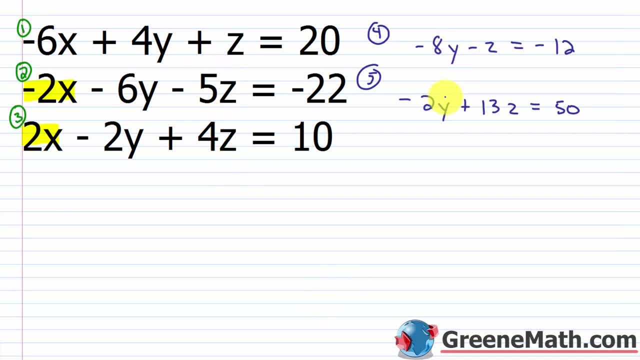 All right, So now I have my linear system in two variables. It looks like this one is easier to solve with substitution. I have a coefficient of negative one there, So let's go ahead and solve this. for z, We have negative eight. y minus z equals negative twelve. 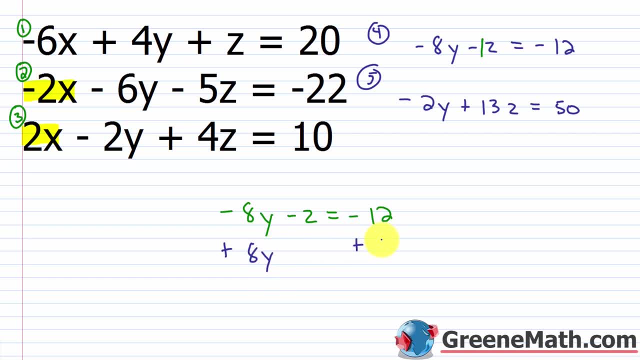 Let's go ahead and add eight y to both sides of the equation. That would cancel. I'll have negative. z is equal to eight y minus twelve. Let's divide both sides by negative one, And so this is going to produce z is equal to negative eight y plus twelve. 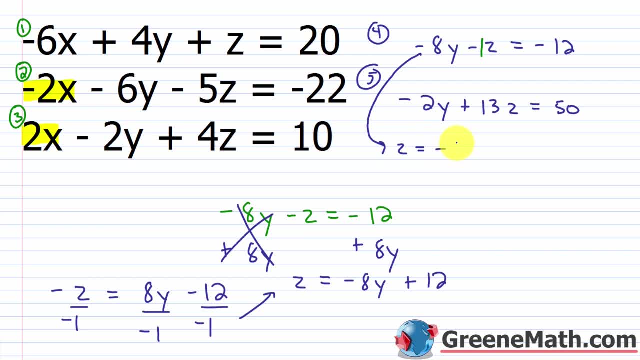 So I'm going to drag this over here. Z is equal to negative eight y plus twelve. All right, So we all know how substitution works. We're going to substitute in for z in this other equation, So I'm going to plug in here and I'm going to be plugging this in. 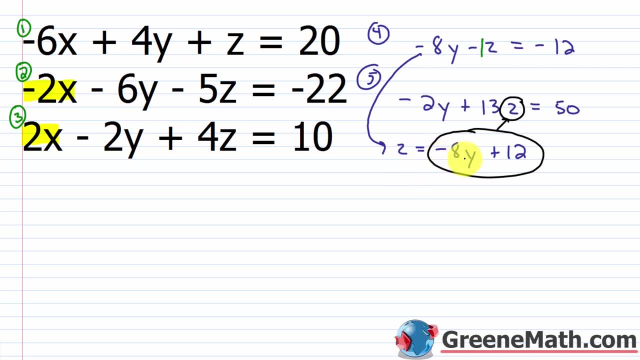 Z equals or z is the same as negative eight y plus twelve. So I'll have my equation five negative two y plus thirteen times. in place of z, I'm going to plug in negative eight y plus twelve, because z is the same as that and this equals fifty. 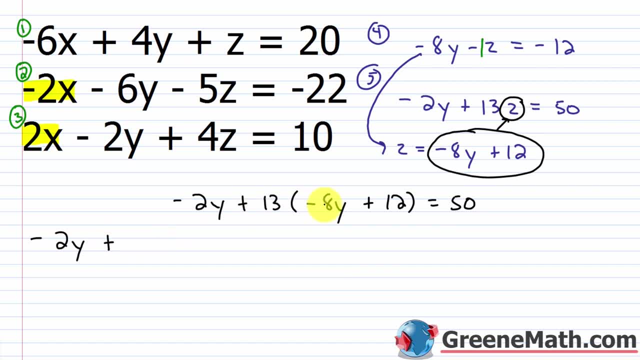 So I'll have negative two y plus thirteen times negative. eight is negative one hundred four. so I can go ahead and put minus one hundred four y and then thirteen times twelve is one hundred fifty six And this equals fifty. So negative two y minus one hundred four y is negative one hundred six y. 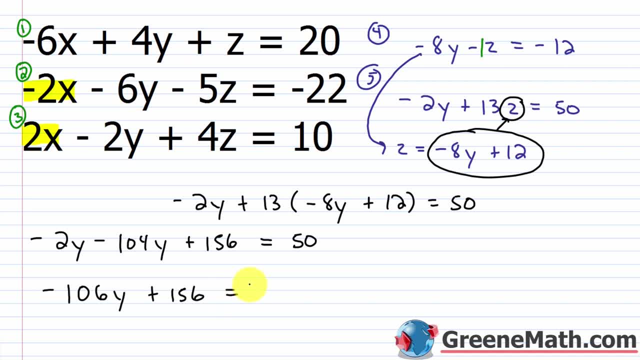 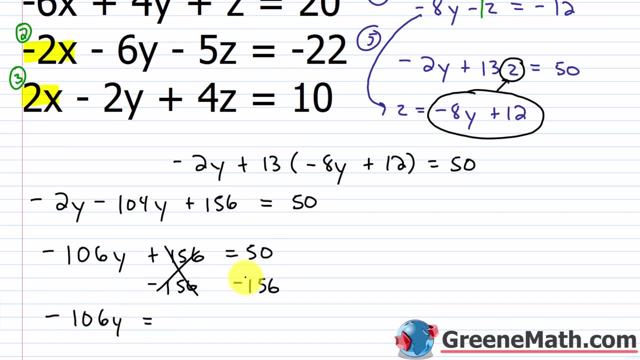 then plus one hundred fifty six and this equals fifty. So if I subtract one hundred fifty six away from each side of the equation, this will cancel. I'll have negative one hundred six. y is equal to fifty minus one hundred fifty six is negative one hundred six. Scroll down and get a little room going. 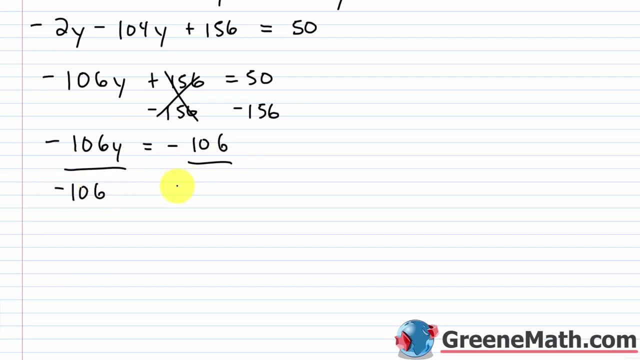 Has a final, Final step. let's divide both sides by negative one hundred six. This will cancel. I'll get: y is equal to negative one hundred six over negative one hundred six is one. So y equals one. So we found one of our unknowns. 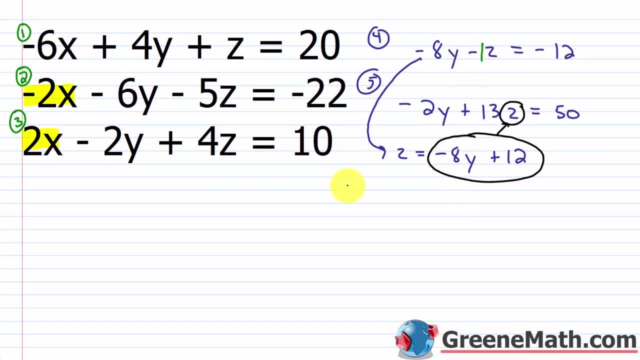 Let me erase everything. So now I'm going to keep working with this linear system in two variables. I'm just going to list that y equals one for now, So I can plug a one back in for y. here or here Doesn't matter, It's easier to work with equation four. 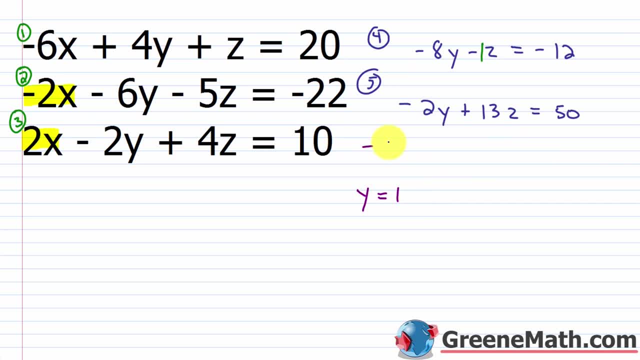 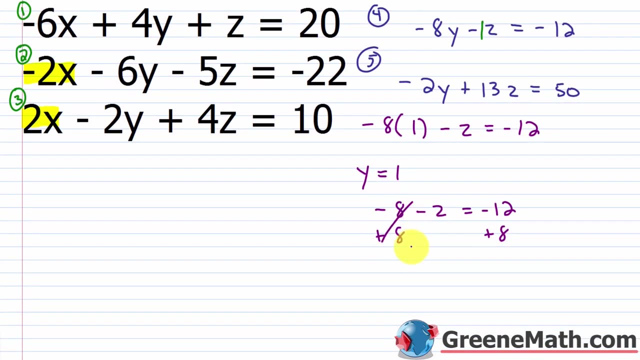 So let's go ahead and do that. So in equation four I'd have negative eight times. Plug in a one for y minus z equals negative twelve. Negative eight times one is going to be negative. eight minus z equals negative twelve. Let's add eight to each side of the equation. that cancels. 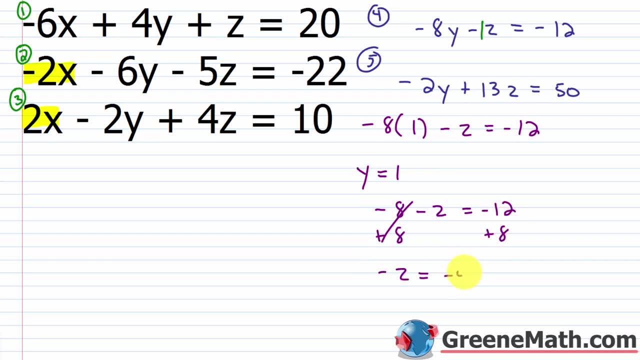 You'll have negative. z is equal to negative. twelve plus eight is negative four. Multiply both sides by negative one, You'll get z is equal to four. So y equals one, z equals four. All right, So now we know two of our unknowns. 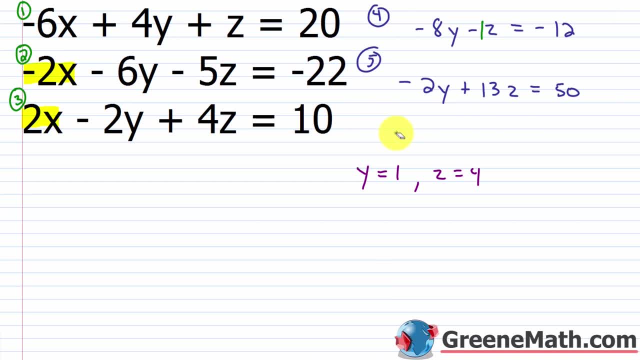 And now we can turn to our original system of equations. So I go back to equation one, two and three. So y equals one in every equation, Z equals four in every equation. So I can plug into equation one, two or three. 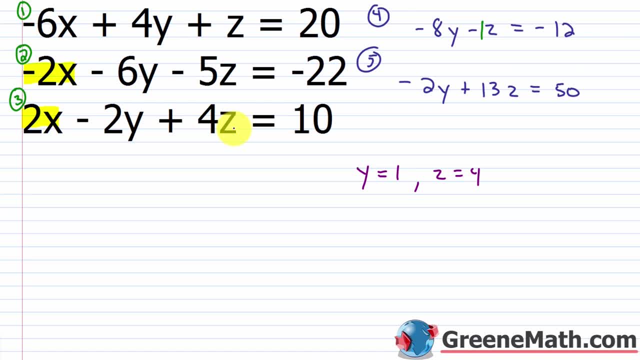 Doesn't matter And find the value of x. So let's just go ahead and work with equation three. So if I have two x minus two, y is one. One plus four times z, z is four. This should equal ten. So I'd have two x minus two plus sixteen equals ten. 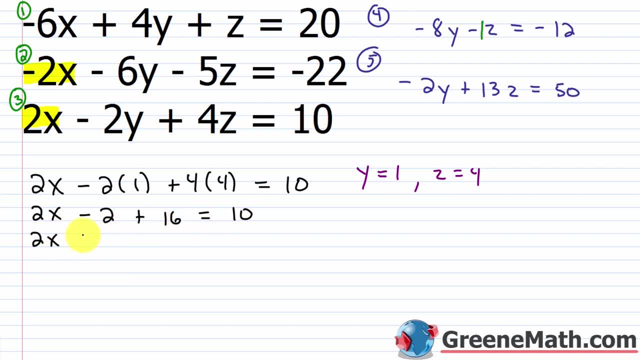 So I'd have two x negative. two plus sixteen is fourteen. This equals ten. Let's subtract fourteen away from each side of the equation. This will cancel. I'll have two. x is equal to ten minus fourteen is negative four. Let's divide each side of the equation by two. 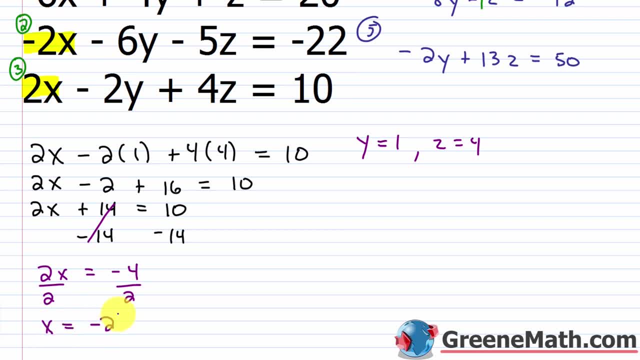 And we'll have: x is equal to negative two. All right, So I found my value for x. X is negative two And let's go ahead and write this as an ordered triple. Remember it's the x value, So that's negative two. The y value. 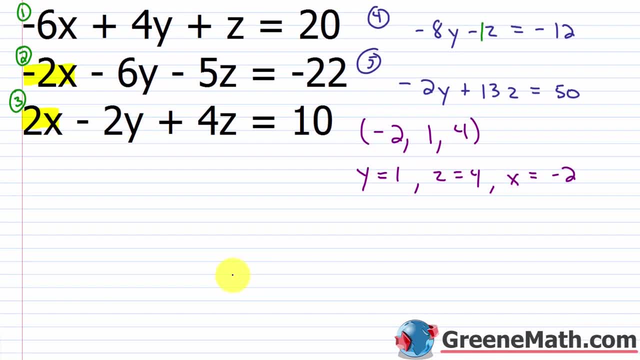 So that's one. The z value is four. So the very last thing we want to do is check. I know checking takes a long time and it's tedious, but it's very important that you check if you have the time, If you're on a timed examination. 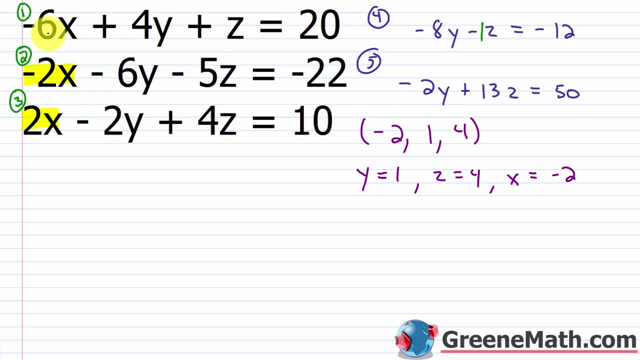 what I always do is, or what I always suggest that you do, would be to go through everything. first, make sure you can complete your test, then go back and check your answers, start with the ones that you think you got wrong And then, if you have time, check everything. 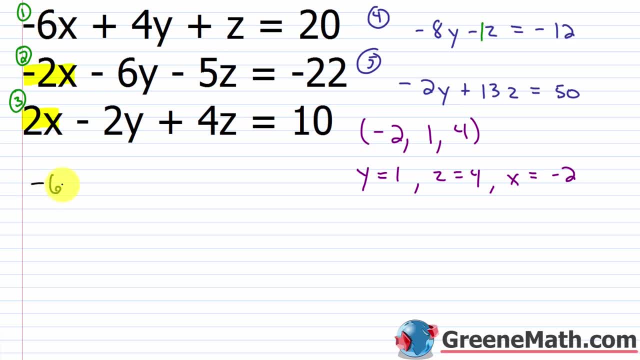 All right, So let's start with equation one. So I would have negative six times for x, I'm plugging in a negative two plus four times for y, I'm plugging in a one plus z, which I'm plugging in a four, four. 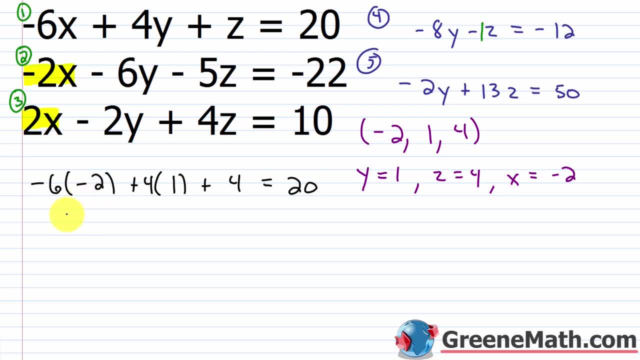 So this should Equal twenty. negative six times negative two is twelve plus four times one is four plus four equals twenty twelve plus four. sixteen sixteen plus four is twenty. So you get twenty equals twenty. So it does work out here For equation two. for equation two we have negative two x. 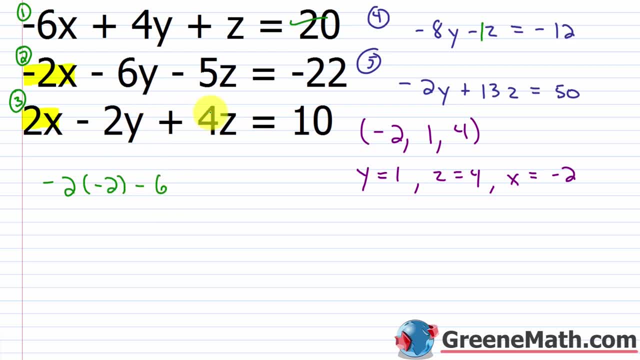 So x is negative two minus six, y. y is going to be one minus five, z, z is again going to be four. This should equal negative twenty two. Negative two times negative two is four minus six times one is six minus five times four is twenty. This should equal negative twenty two. 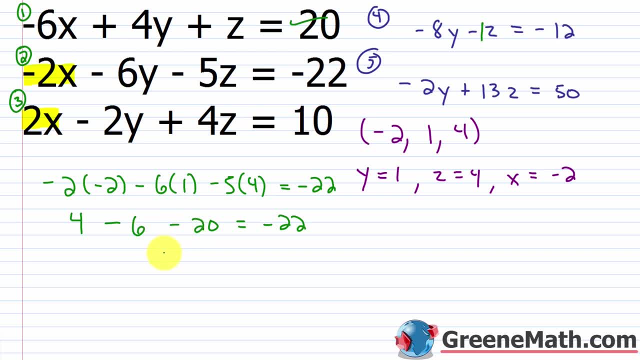 Four minus six is negative two Negative. two minus twenty is negative twenty two. You get negative twenty two equals negative twenty two, So it works out here as well. Let's check equation three. So we'd have two times x. X is negative. two minus two times y. 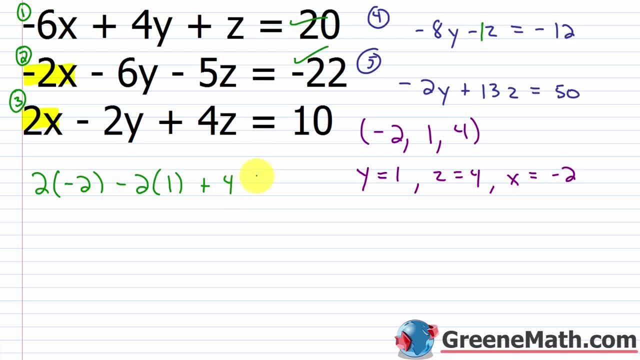 Y is one Plus four times z, Again z is four. So this equals ten Two times negative. two is negative. four minus two times one is two plus four times four is sixteen. This should equal ten. Negative. four minus two is negative six. 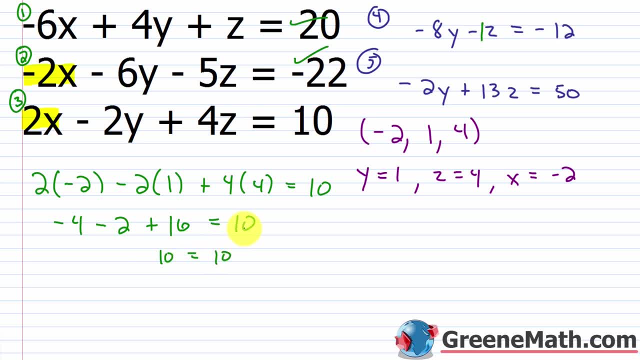 Negative six plus sixteen is ten, So you get ten equals ten, So it works out here as well. So we found our solution for our system. It took a while, but we did find it. It's the ordered triple negative: two comma one comma four. 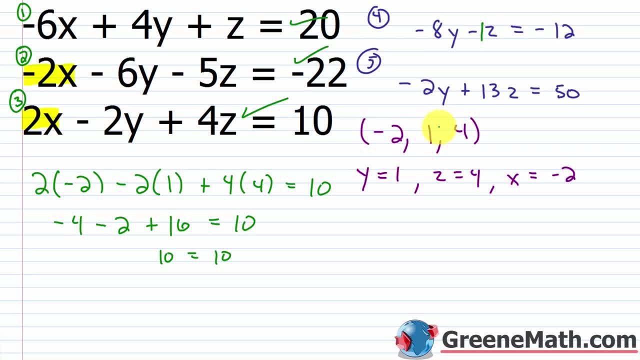 Which is an x value of negative two, a y value of one, a z value of four. Now I'm not going to check everything moving forward just for the interest of time, because it takes forever, But I want you guys to pause the video just so you know how to check things. 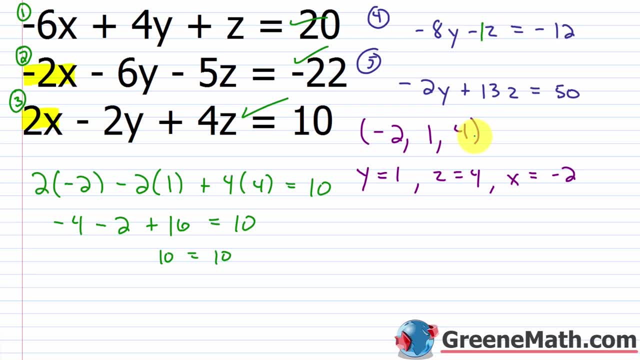 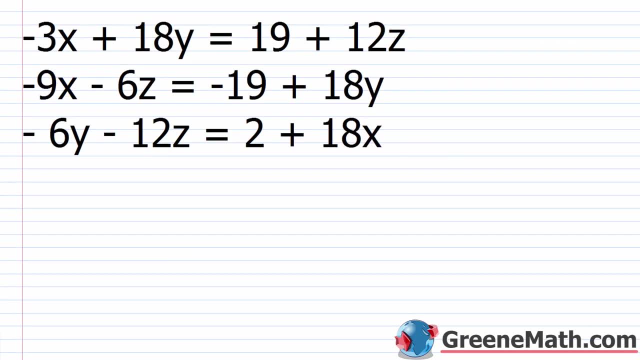 Plug in for every x, plug in for every y, plug in for every z and make sure all of the equations are true with our solution. All right, let's go ahead and take a look at the next example. We're going to kind of speed things up just a little bit. 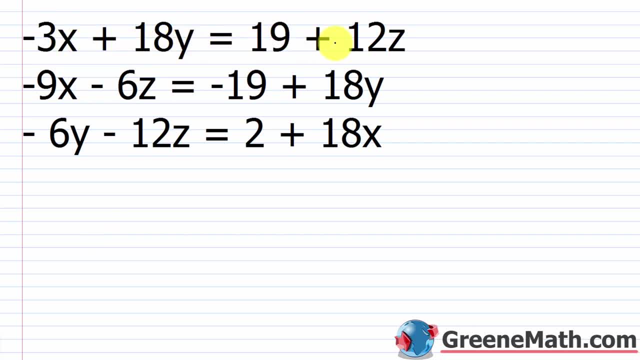 So I have negative three x plus eighteen y equals nineteen plus twelve z. I have negative nine x minus six z equals negative nineteen plus eighteen y. I have negative six y minus twelve z equals two plus eighteen x. Now, this is not in the format that we'd like it in. 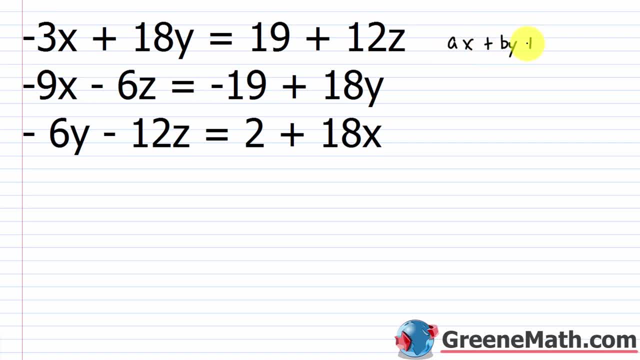 We want it in ax plus by plus cz equals k. Do we have to have it in this format? No, but it makes it convenient for us to see what's going to cancel, what we need to do to cancel. We don't want to be looking all over the place to find z and x and all these things. 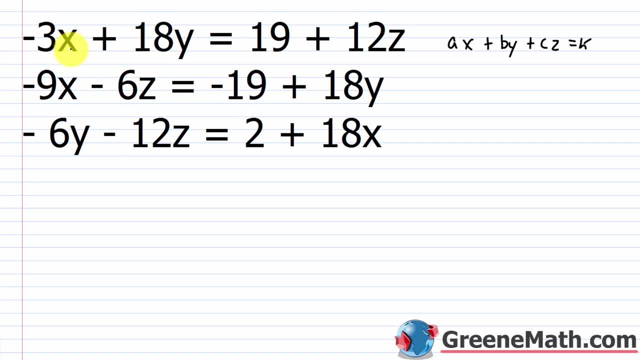 We want things lined up nice and neat. So for the first equation I'm going to write negative three x plus eighteen y. If I subtract twelve z away from each side, I can put minus twelve z over here, and this would be equal to nineteen. 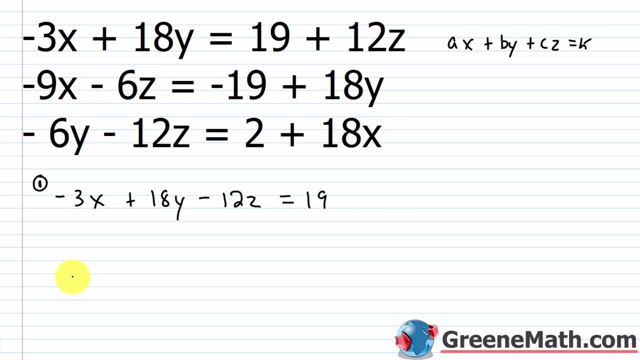 So this would be my equation one. For equation two, I have negative nine x. I could subtract eighteen y away from each side, then minus six z, And this equals negative nineteen. OK, this is my equation two. For equation three, let's subtract eighteen x away from each side of the equation. 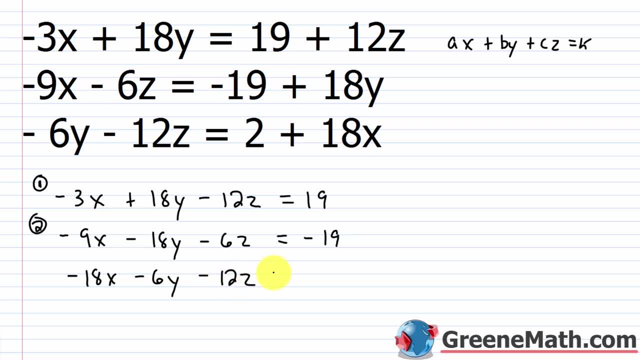 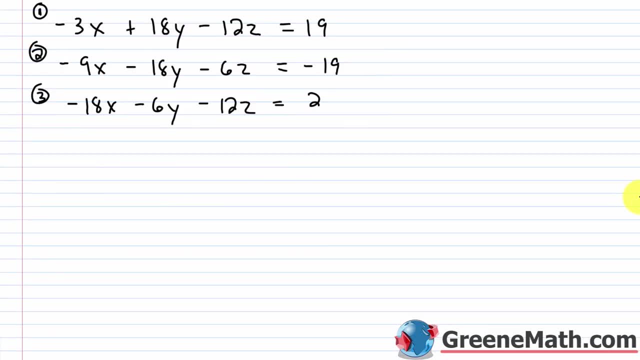 Then minus six y, then minus twelve z, and this equals two. So this would be my equation three. All right, so let's scroll down and let's go ahead and eliminate one of the variables from two of the equations. Now, looking at this again, everything's nice and neat laid out for me. 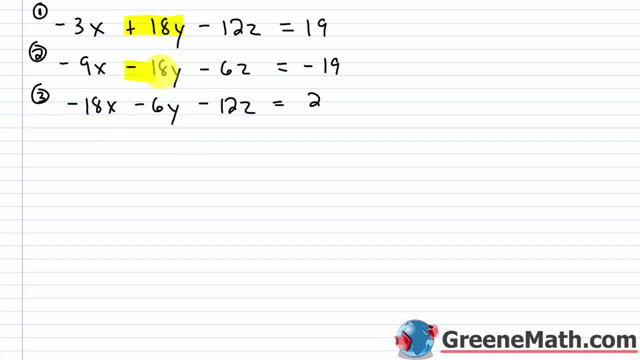 I can see that I have plus eighteen y and minus eighteen y. So let's go ahead and start with what's easy. Let's take equation one and equation two and let's eliminate the variable y, So we have negative three x plus eighteen y, minus twelve z equals nineteen. 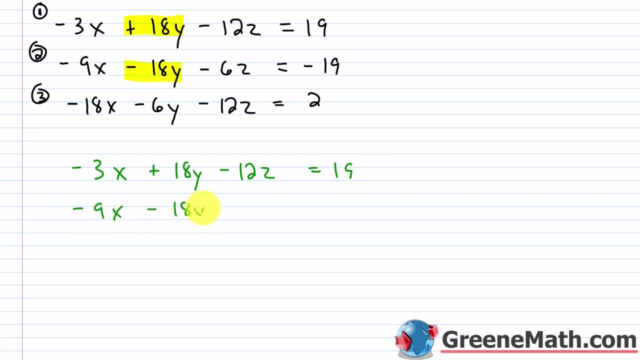 We have negative nine x minus eighteen y Minus six z equals negative nineteen. All right, so if I add the left sides together and I set this equal to the sum of the right sides, negative three x minus nine x is negative twelve x. 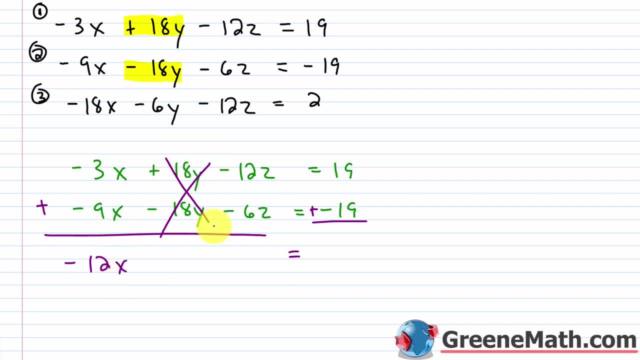 Eighteen y minus eighteen y is zero, So y is eliminated. Negative twelve z minus six z is minus eighteen, z. Nineteen plus negative nineteen is zero. So I'm going to write equation four here as negative. twelve x Minus eighteen z equals zero. 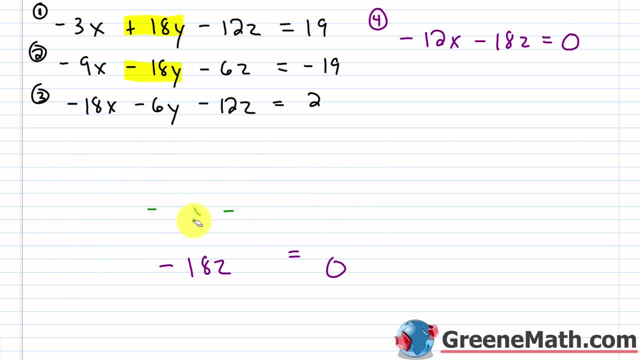 All right. So now what I need to do is pick two other equations and again eliminate the same variable, y. So let's go ahead and work with equation one and equation three. So for equation one I have negative three x plus eighteen, y minus twelve, z equals nineteen. 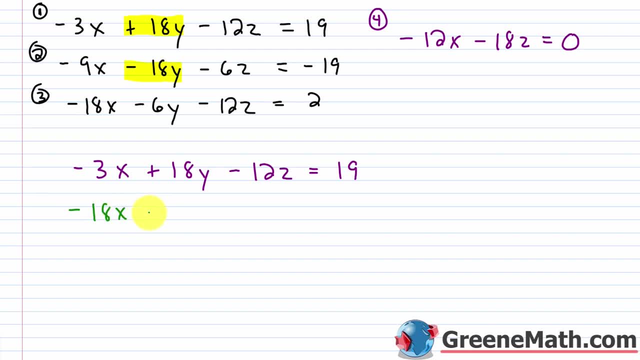 For equation three, I have negative eighteen. x minus six, y minus twelve z equals two. Now if I want these to be opposites, I need to multiply negative six by three. But I've got to multiply both sides of the equation by three to make that legal. 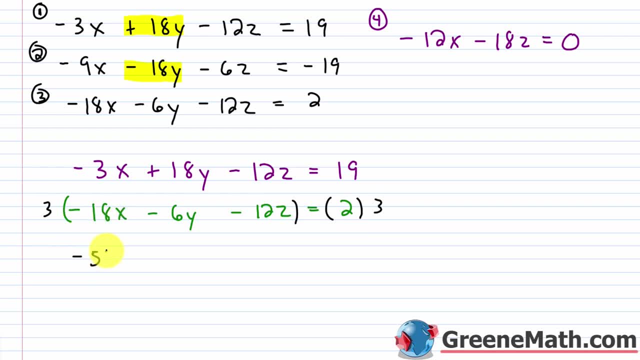 Three times negative. eighteen x is negative. fifty four x Minus three times six, y is eighteen y Minus three times twelve. z is thirty six z, And this equals three times two, which is six. All right, let's bring this up now. 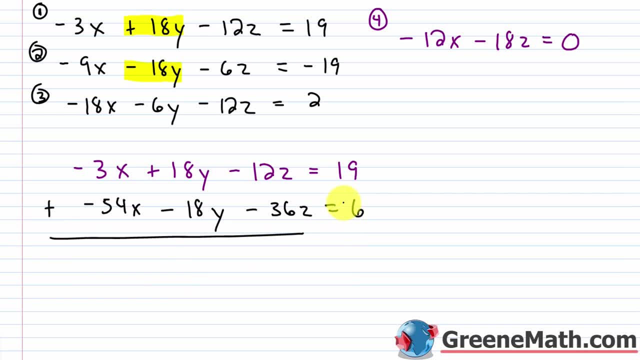 So let's add the left sides together. Set it equal to the sum of the right sides. Negative: three x minus fifty four. x is negative. fifty seven x. Eighteen y minus eighteen. y is zero. Y is eliminated. Negative: twelve z minus thirty six. z is minus forty eight z. 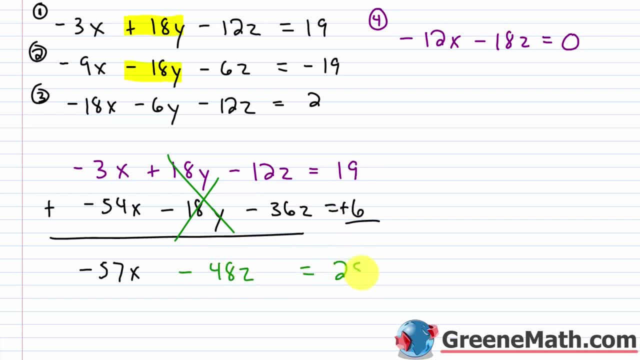 Then this equals nineteen plus six, which is twenty five. All right, so let's put this as equation five here. So we have negative. fifty seven x Minus forty eight z equals twenty five. So now I have a linear system in two variables. 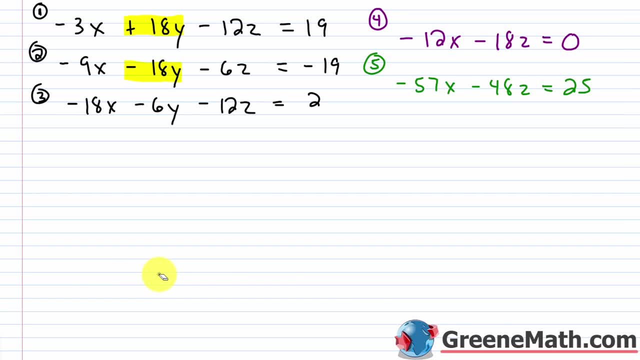 So what I can do is again solve that I can use elimination or substitution, really whatever I want. So it looks like I'm going to use elimination here, So I'm going to choose to eliminate the variable z. So how would I do that? if I have negative twelve x minus eighteen, z equals zero, and 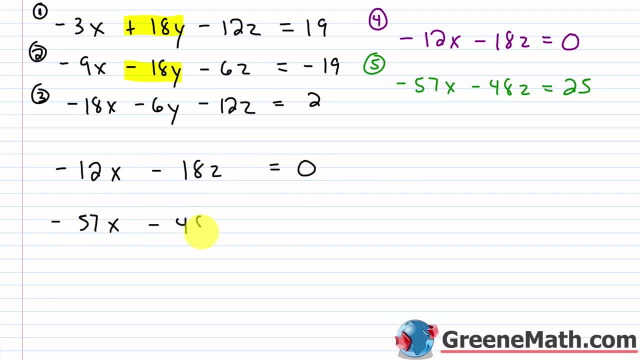 I have negative. fifty seven x minus forty eight z equals twenty five. What's the least common multiple between eighteen and forty eight? So the LCM of eighteen and forty eight? Well, I know, eighteen is six times three. So two times three times three, What's forty eight? 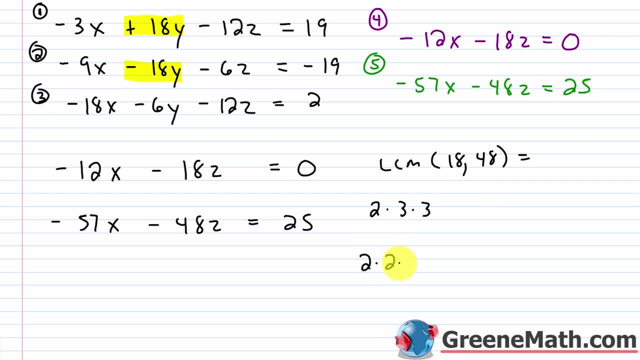 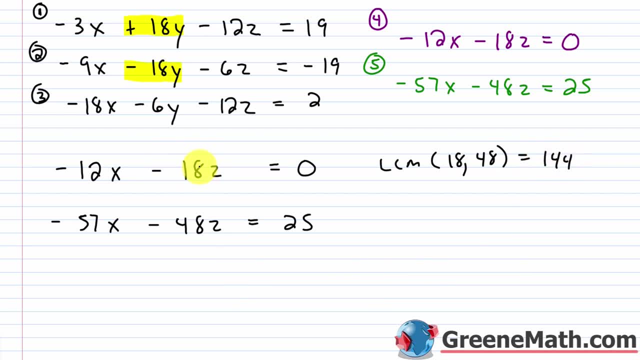 One hundred forty four. So I want one of these to be negative one hundred forty four z, the other to be positive one hundred forty four z. So let's multiply this equation, both sides, by negative eight. And then let's multiply both sides of this equation. 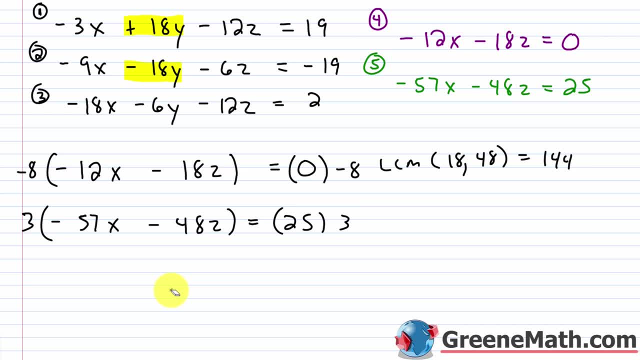 by positive three, So I would have negative eight times negative twelve x, That would be ninety six x, Then negative eight times negative. eighteen z would be positive one hundred forty four z, and this equals zero times negative eight, which is zero. Next we have three times negative fifty seven x. 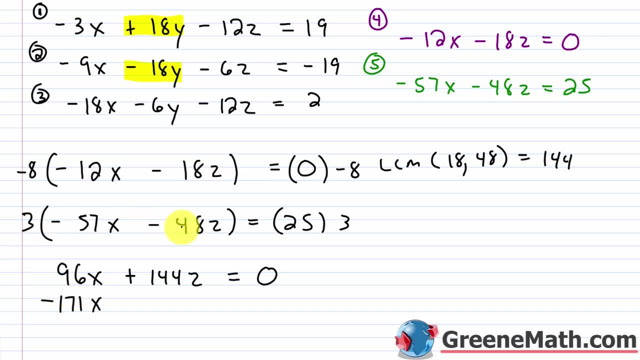 That's negative one hundred seventy one x, Then three times negative forty eight z. That's going to give me negative one hundred forty four z. This equals three times twenty five, seventy five. All right, so let's erase this. I don't need any of this anymore and I'm going to drag this up a little bit. 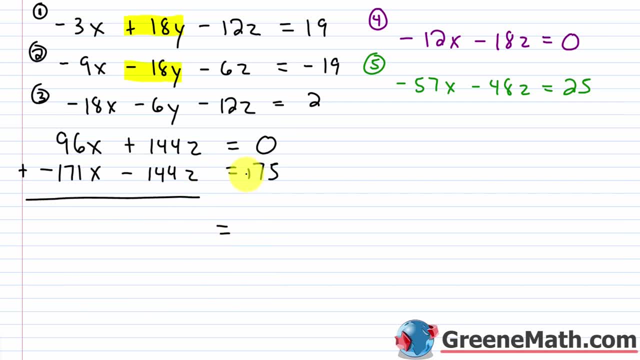 So if I add the two left sides together and set it equal to the sum of the right sides, what am I going to get? Ninety six x plus negative one hundred seventy one x is going to give me negative seventy five x. one hundred forty four z minus one hundred forty four z is going 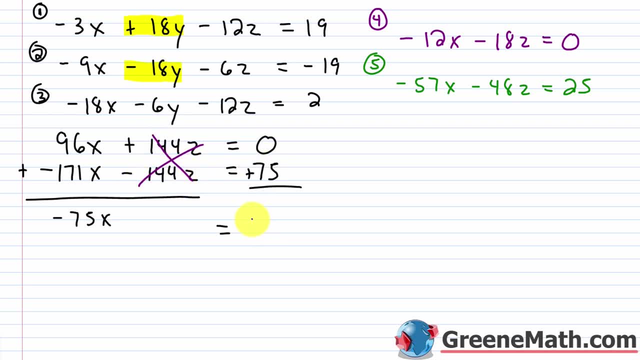 to be zero, right. So z is eliminated. Zero plus seventy five is seventy five, So I get negative seventy five. x equals seventy five. I divide both sides by negative seventy five and I get that x is equal to negative one. x is equal to negative one. 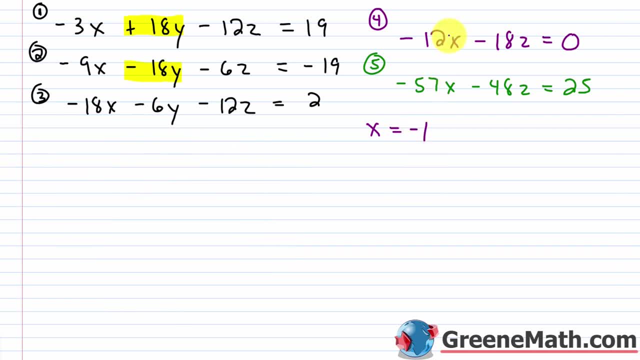 OK, let's erase all this. Now, if I stay with this system in two variables, I'm going to find out what z is. So let's plug into equation four. We have negative twelve times for x. I'm going to plug in a negative one. 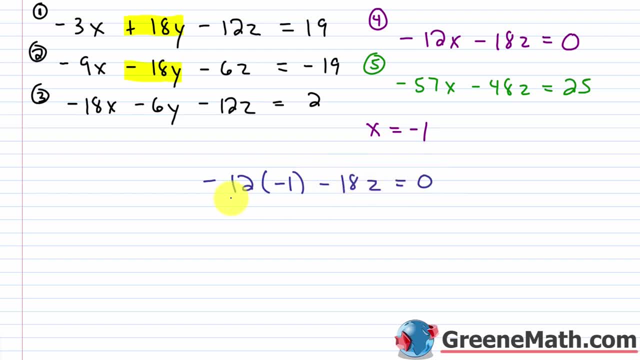 Minus eighteen times z equals zero. Negative twelve times negative one is twelve. So we get twelve minus eighteen z equals zero. I would subtract twelve away from each side of the equation. That's gone, I'll have negative. eighteen z is equal to negative twelve. 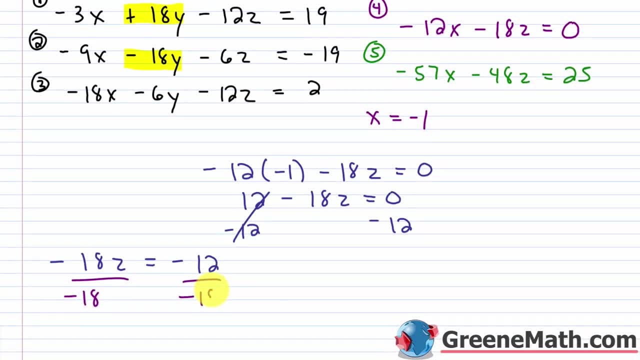 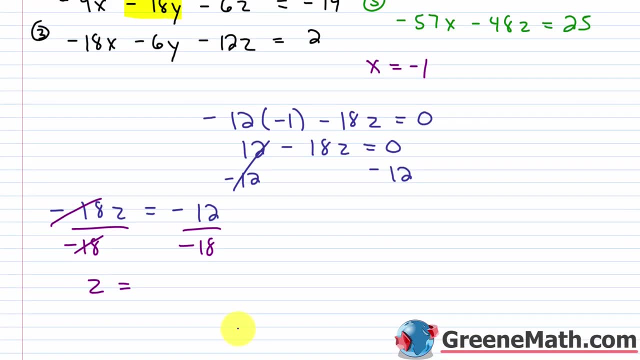 Let's divide both sides of the equation by negative eighteen, So that'll cancel, I'll have. z is equal to. we know negative over negative is positive. But we think about Twelve and eighteen. Each is divisible by six. Divide twelve by six. 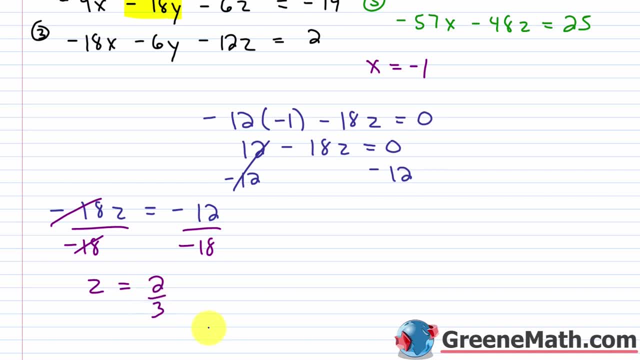 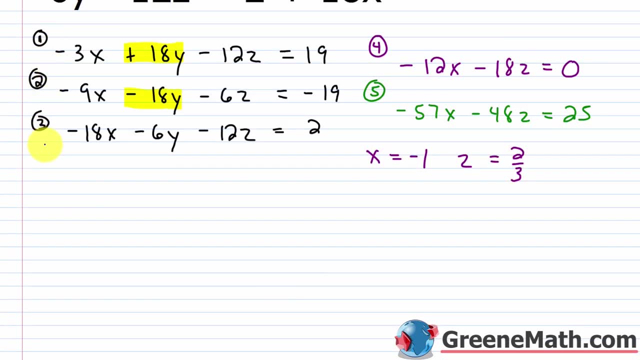 You get to divide eighteen by six, You get three. So z is going to be two thirds. So now let's look at our equations that have three variables. I'm going to take one of them, Doesn't matter which one. Plug in a negative one for x. plug in a two thirds for z. 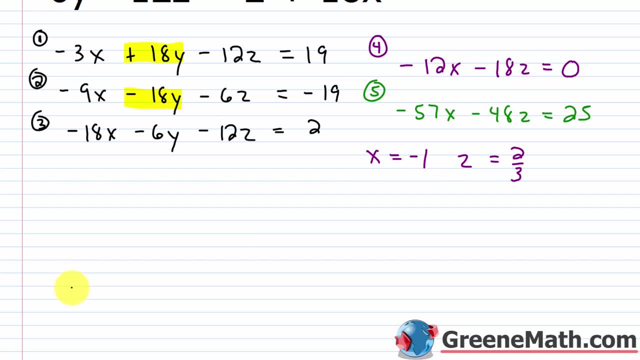 I'm going to find out why. So let's go ahead and work with equation number one. So you'd have negative three times Again. x is negative one plus eighteen, y minus twelve times z. Z is two thirds, And this equals nineteen. 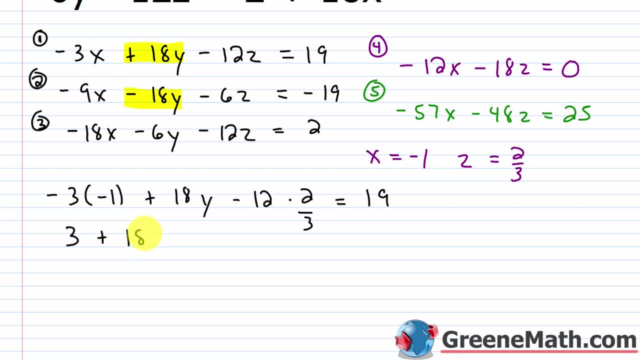 Negative three times negative. one is three plus eighteen y Negative twelve times two. thirds Twelve would cancel with three and give me four. So really I have negative four times two, which is negative eight. This equals nineteen. Three minus eight is negative five. 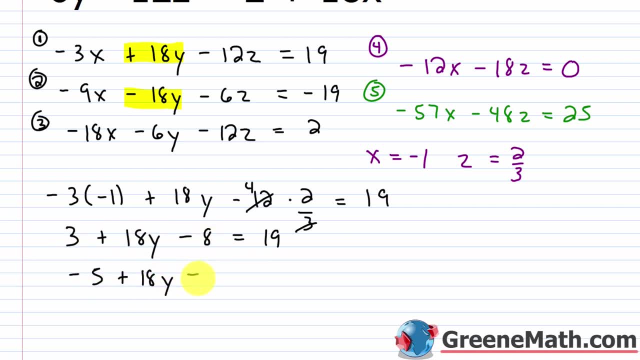 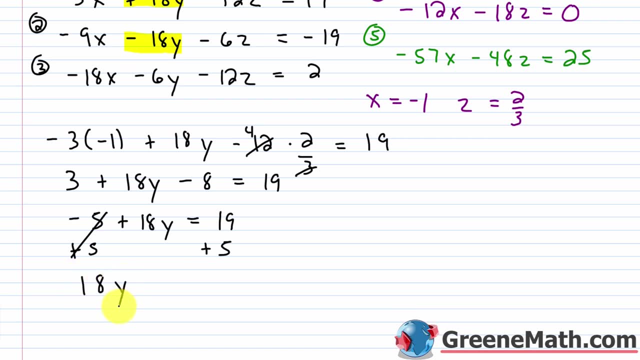 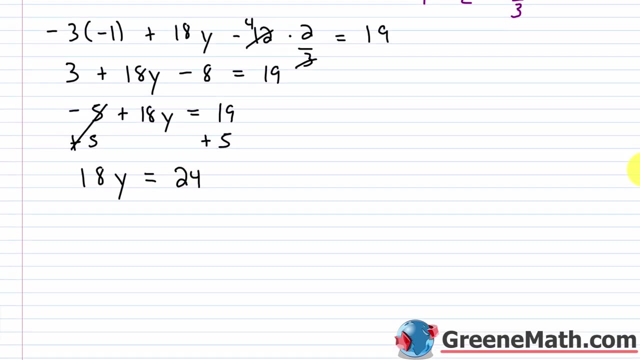 So you'd have negative. five plus eighteen y Is equal to nineteen. Add five to each side of the equation. That would cancel. You'll have eighteen. y is equal to nineteen plus five is twenty four. Now to get y by itself, let's divide both sides of the equation by eighteen. 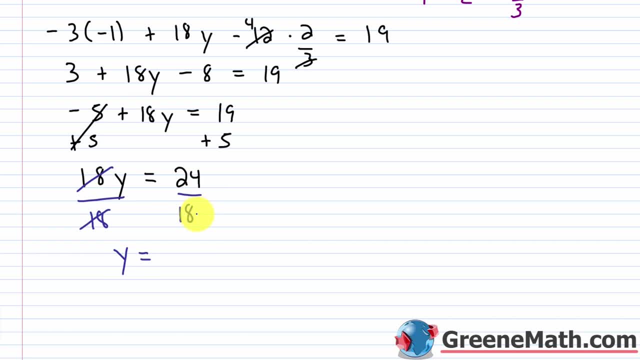 This will cancel. with this I'll get: y is equal to twenty. four and eighteen are each divisible by six. Twenty four divided by six is four. Eighteen divided by six is three, So y is going to be equal to four thirds, So y is equal to four thirds. 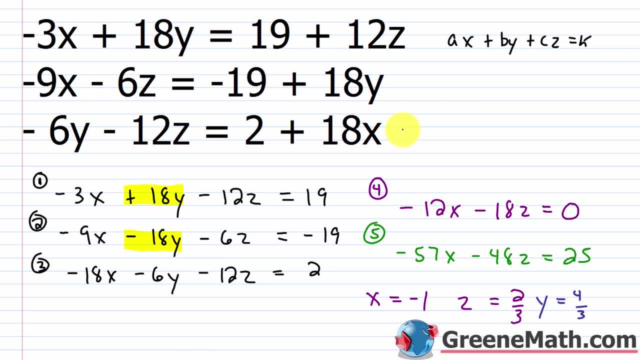 So, as an ordered triple, as an ordered triple Again, it's the x value which is negative one, The y value, which is four thirds, and the z value, which is two thirds. So that's going to be your solution to this system. 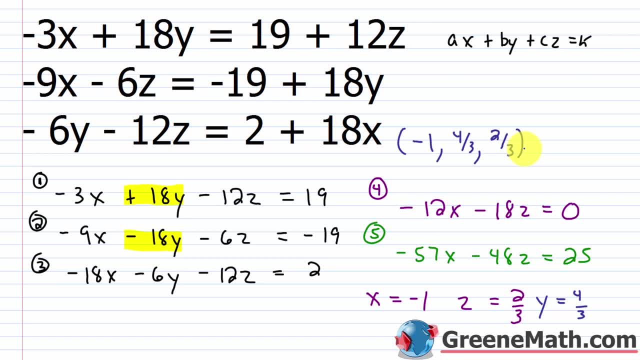 In the interest of time, I'm not going to go through and check it, But I want you to pause the video. if you're unsure how to do it, Plug in a negative one for every x, A. four thirds for every y, A. two thirds for every z. 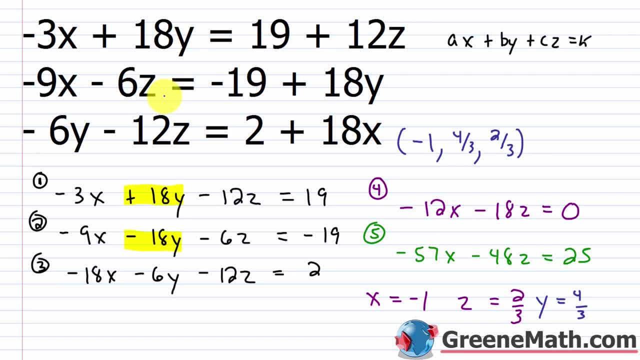 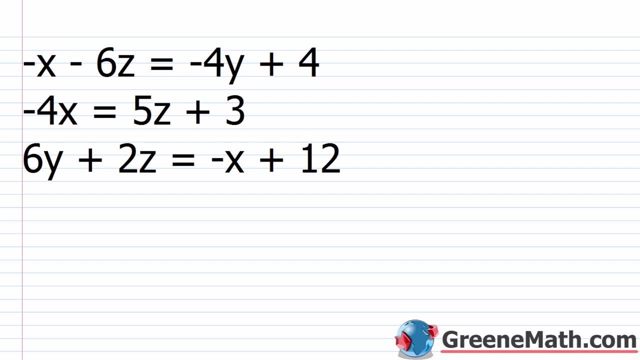 And make sure the left and the right side are equal in each of the three equations. Alright, let's take a look at another one. So we have negative x minus six z equals negative four y plus four. We have negative four x equals five z plus three. 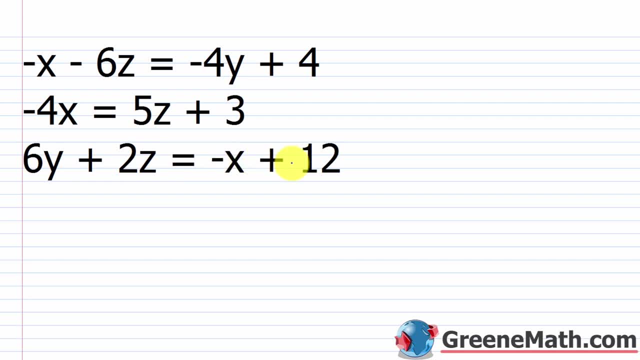 We have six y plus two. z equals negative x plus twelve. So a lot of students see this and they go. well, you're missing a variable in the second equation. That's OK. I'm going to show you how that's going to actually be a benefit to you. 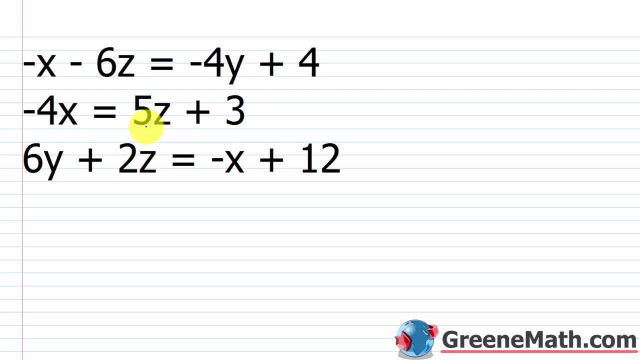 And it's going to take less time to do a problem like this. The first thing is I want to write every equation in this format: A x plus b, y plus c, z equals k. So for this top equation, negative x, add four y to each side. 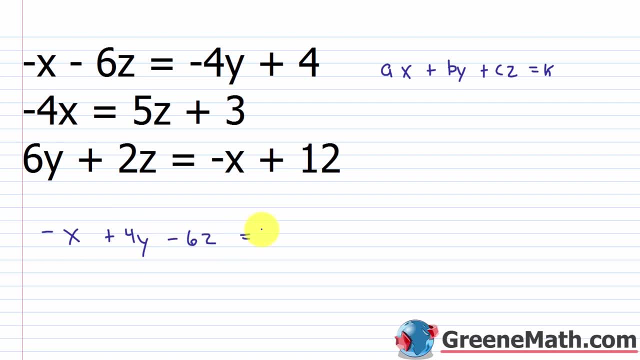 So plus four y minus six z equals four. For the next equation, negative four x. I don't have a y, so I can put plus zero y if I want, And then I'm going to subtract five z away from each side, and this equals three. 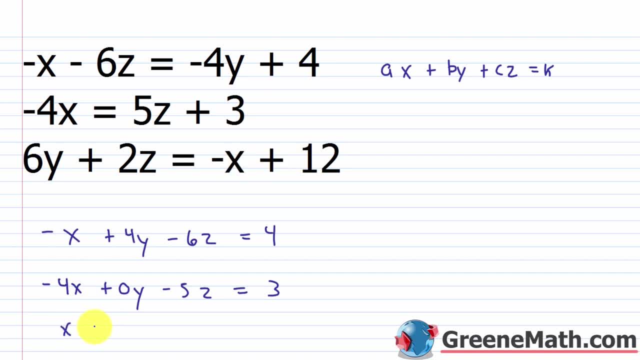 For the third equation, I'll add x to each side of the equation, And then plus six y, plus two z, and this equals twelve. So, just as I always do, I'm going to number these. This is equation one, two and three. 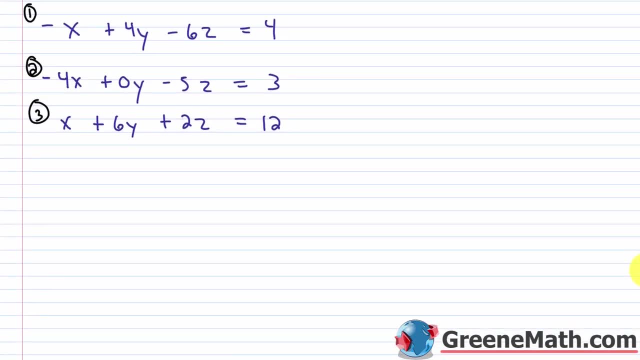 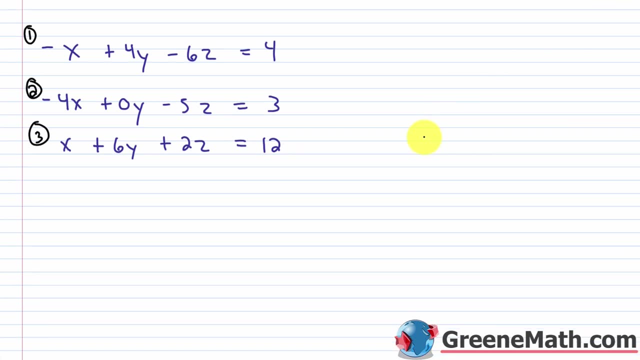 All right, now let's talk about how this is an improvement for us. One thing is: normally I have to eliminate one of the variables from any two equations. Then I've got to do that again. I've got to eliminate the same variable from another two equations. 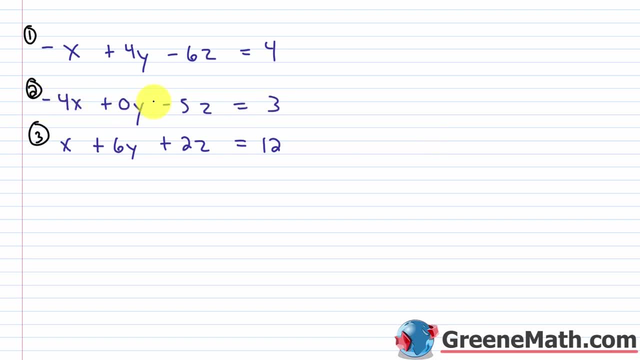 I noticed that this equation does not have a y. It's got zero y. You can basically just take y out. So I'm just going to write this over here as negative. four x minus five z equals three. If I just take equation one and three and I 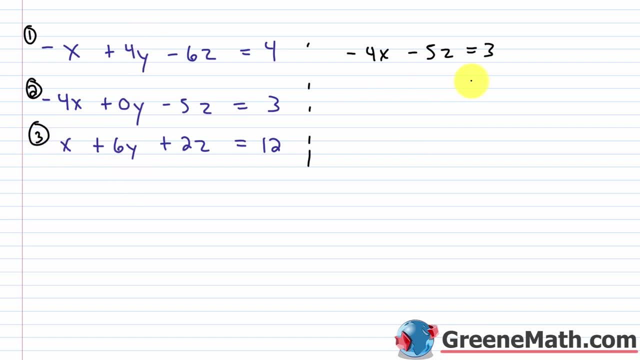 eliminate y. I can write this over here as an equation with x and z only, And I can basically have a linear system with two variables and I can get my solution very quickly So I can skip a step when this occurs. So with equation one and three I have negative x plus four, y minus six, z equals. 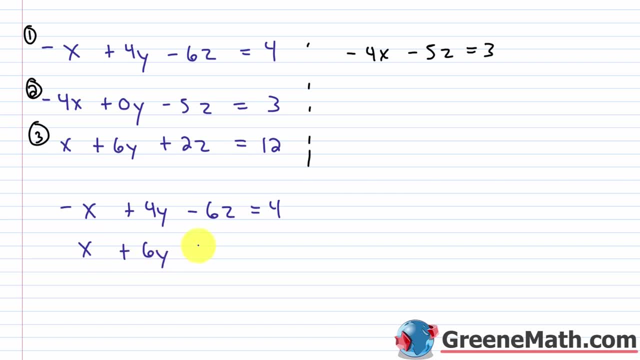 four and I have x plus six, y plus two, z equals twelve. Now I know some of you look at that and say: oh, I've got negative x and x. Let's just go ahead and eliminate x. That's not going to do you any good, because over here you have x and z. 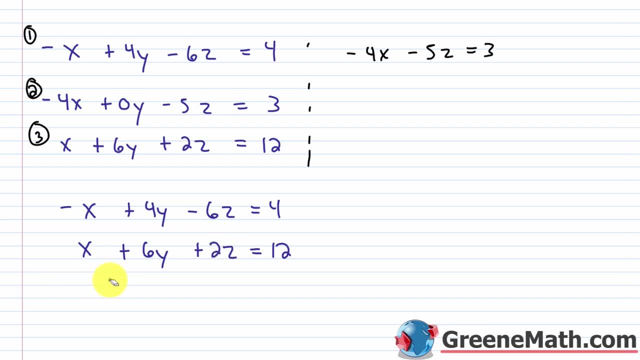 If I eliminate x and have y and z, I need a linear system with the same two variables. OK, so don't think like that, All right. So the first thing I want to do is think about how I can get four y and six y into opposites. 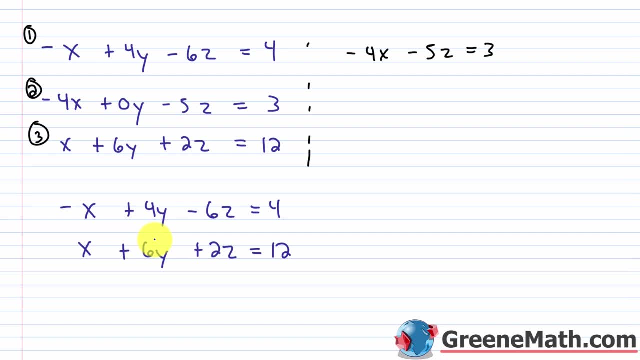 Well, you think about the least common multiple between the two, and it would be twelve. So I want one of them to be twelve. Why The other to be negative twelve? Why? So I can multiply both sides of this equation by, let's say, negative three. 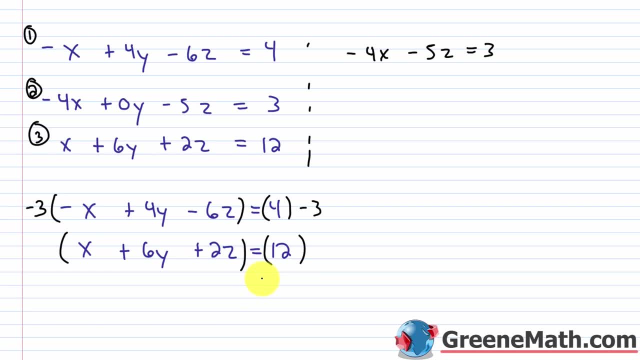 And I can multiply both sides of this equation by, let's say, positive, two. So negative three times negative. x would be three x. Negative three times four: y would be minus twelve y. Negative three times negative: six z would be plus eighteen z. 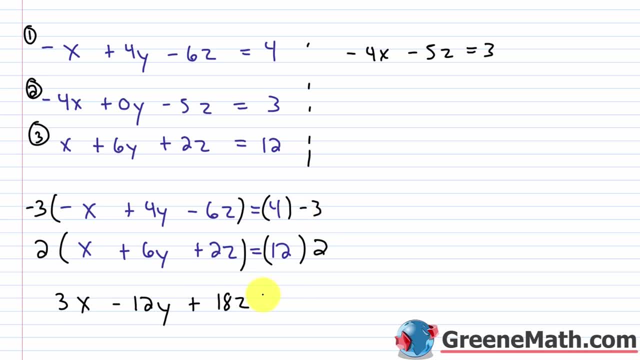 Negative. three times four would be negative twelve. So this equals negative twelve. Two times x would be two x. Two times six y would be plus twelve y. Two times two z would be four z. And this equals two times twelve, which is twenty four. 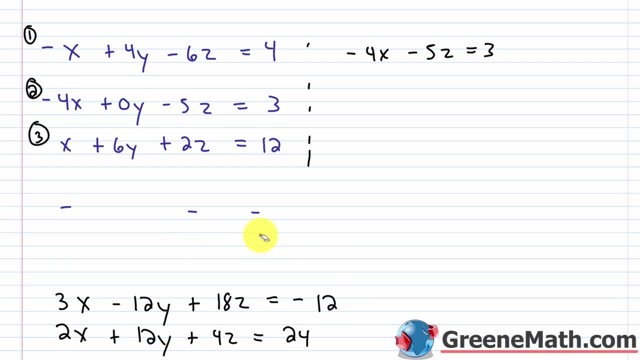 All right, So let me erase this. I don't need this anymore- And we're ready to add the two left sides together. Set that equal to the sum of the two right sides. So what's that going to give me? Three x plus two x is five x. 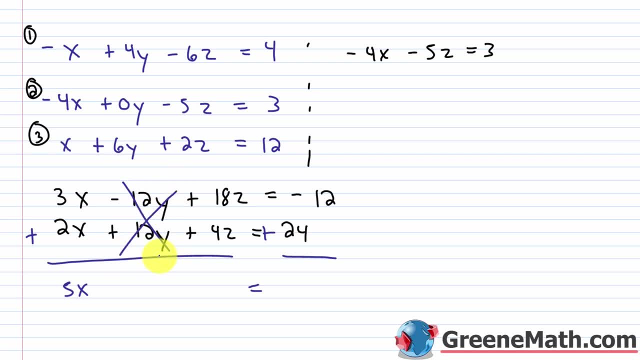 Negative twelve y plus twelve. y is zero, So y is eliminated. Eighteen z plus four z is twenty two. z. This equals negative twelve plus twenty four, which is twelve. So I've got another equation here. This is equation two, so I'll keep that number. 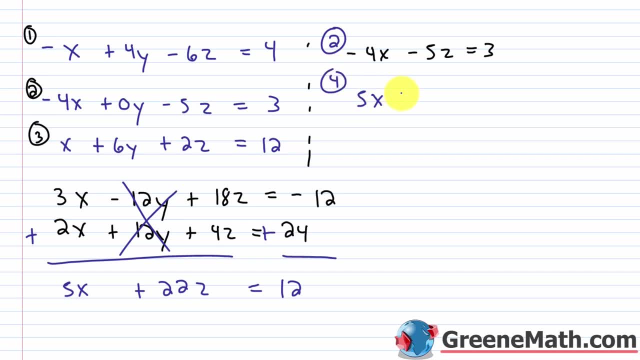 This will be equation four. It's five x plus twenty two. z equals twelve. All right, So now we can just solve for x and z and then plug back into one of the original equations. So the easiest thing to do, I think, in this case would be to use elimination. 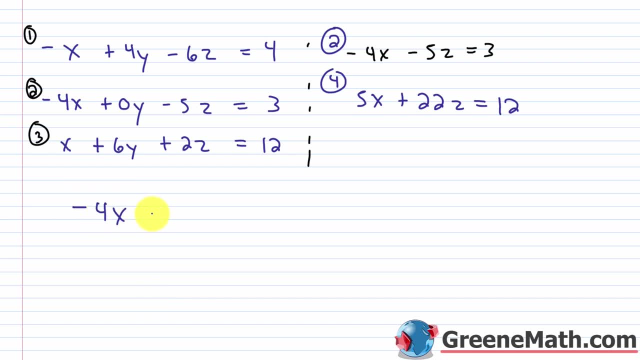 If I have negative four x minus five, z equals three, and I have five x plus twenty two, z equals twelve. Between negative four and five, the LCM is twenty. So I can make one of them positive twenty, one of them negative twenty, and I'm going to be good to go. 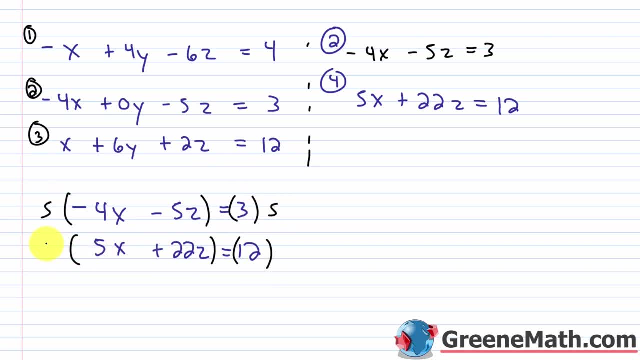 So I'm going to multiply both sides of this by five and both sides of this by four. So five times negative four x is negative twenty x. Five times negative five z is minus twenty five z. Five times three is fifteen, So this equals fifteen. 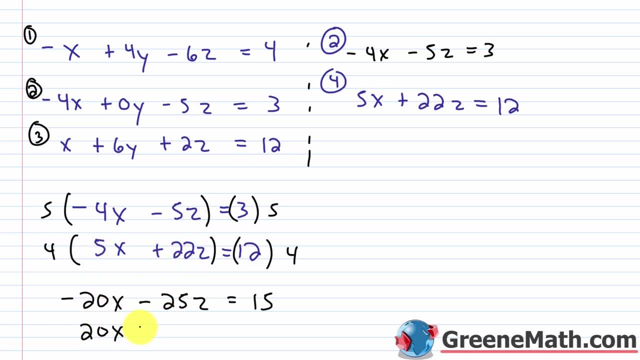 Four times five, x is twenty x. Four times twenty two, z is plus eighty eight, z. This equals four times twelve is forty eight. Let's erase this. So let's bring this up. All right, So let's sum the two left sides. 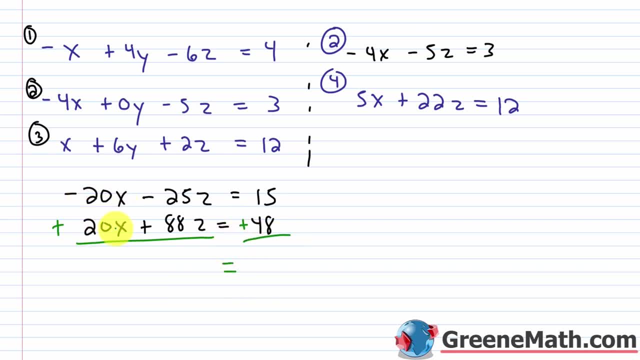 Set this equal to the sum of the right sides. Negative twenty x plus twenty x is zero. Negative twenty five z plus eighty eight z is sixty three z, And this is equal to fifteen plus forty eight is sixty three. So divide both sides of the equation by sixty three. 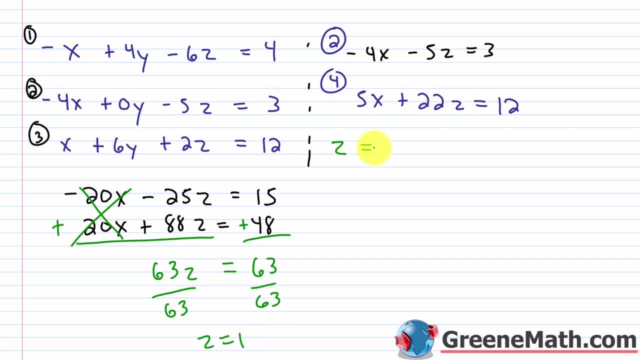 You get that z is equal to one. So z here equals one. So I can plug a one back in for z in either equation two or four, Doesn't matter, Let's go ahead and use equation four. So five x plus twenty two times one. 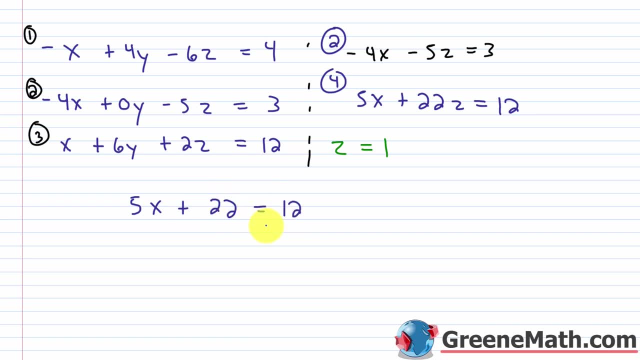 Twenty two times one is just twenty two. This equals twelve. Let's subtract twenty two away from each side of the equation. This is going to cancel. You'll have five. x is equal to twelve minus twenty two is going to be negative ten. 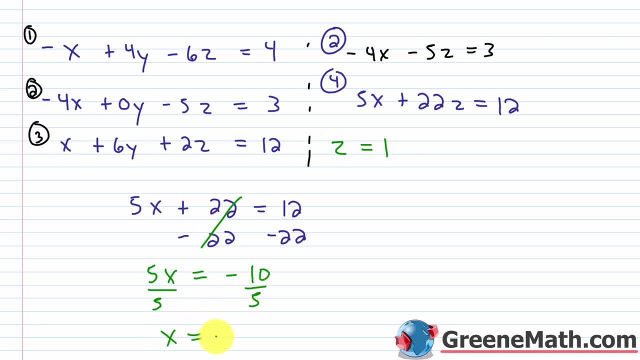 Let's divide both sides of the equation by five, We'll get: x is equal to negative two, So x equals negative two. Now we can take these values, plug them back in for either equation one or equation three and get a value for y. We can't do that with equation two because y 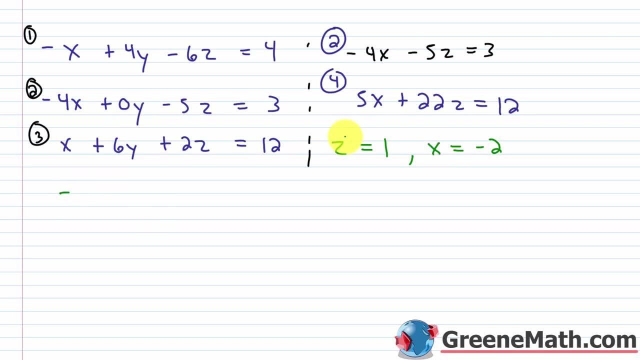 isn't there. So in equation one I can go minus a negative two. Plug in a negative two for x Plus four, y minus six, z, This is one. So minus six times one, This equals four. So minus a negative two is two. 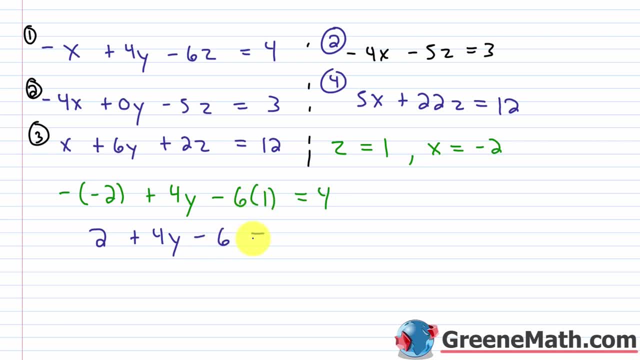 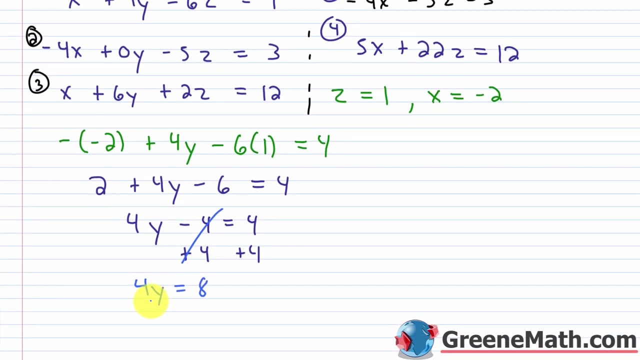 Plus four, y minus six times one, which is six, And this equals four. Two minus six is negative four, So you get four. y minus four equals four. When add four to each side of the equation, this will cancel. You'll have four. y is equal to eight. 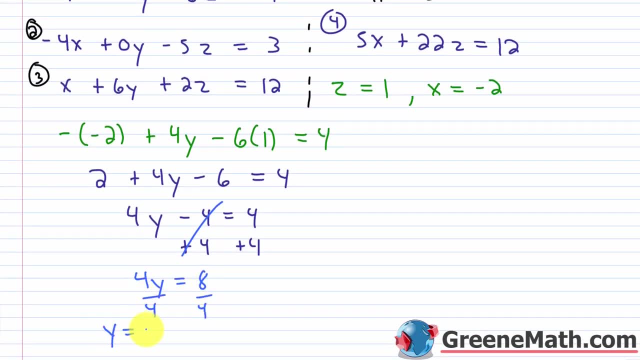 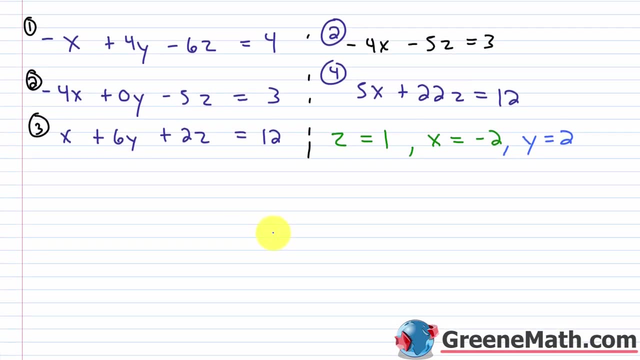 Divide both sides of the equation by four, You're going to get that y is equal to two. OK, so y is equal to two. Let's erase all this. We'll write this as an order triple, So it's the x value which is negative two. 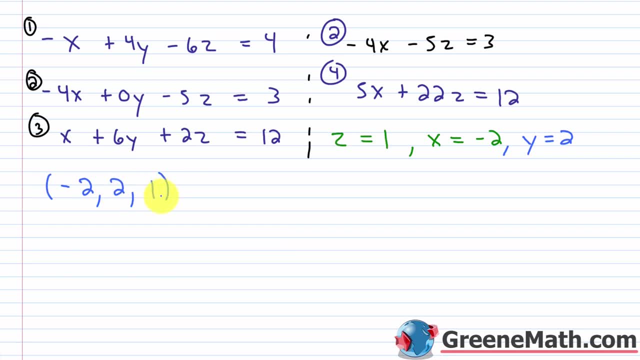 The y value, which is two, Then the z value, which is one. So negative two comma, two comma one. Or an x value of negative two, a y value of two, a z value of one. That's your solution for this system. 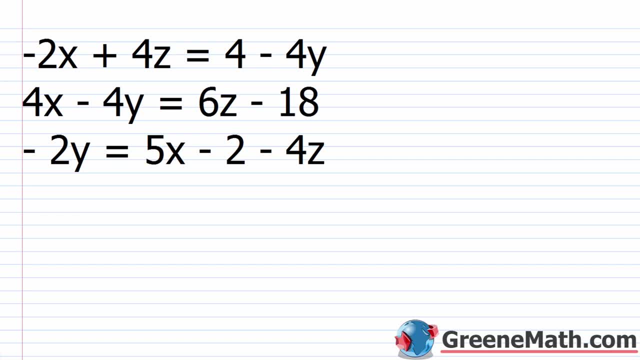 All right. So let's look at one final problem, And I know these get super, super tedious. You know, when you start working through stuff like this, you can go through an hour's worth of work and it can be only like five or six problems. 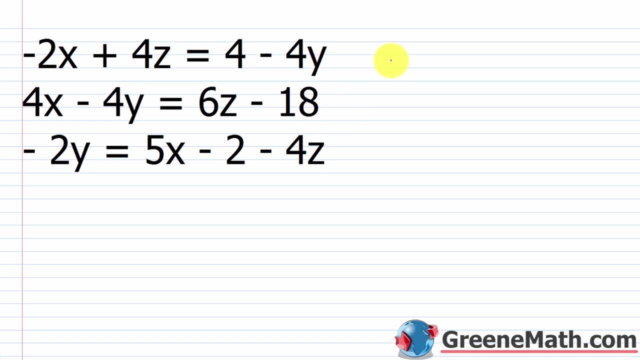 So let's go ahead and start out by just rewriting everything as ax plus by plus cz equals k. For the first equation I have negative two x, negative two x. I'm going to add four y to each side. So plus four y, then plus four z. 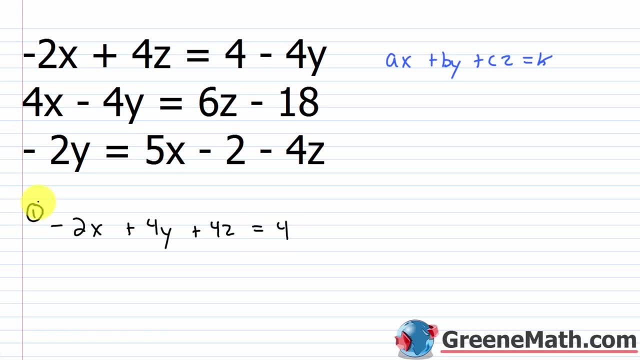 And this equals four. So let's go ahead and call that equation one. For the next equation, we'd have four x minus four y. Let's subtract six z away from each side. This equals negative 18.. Let's call this equation two. 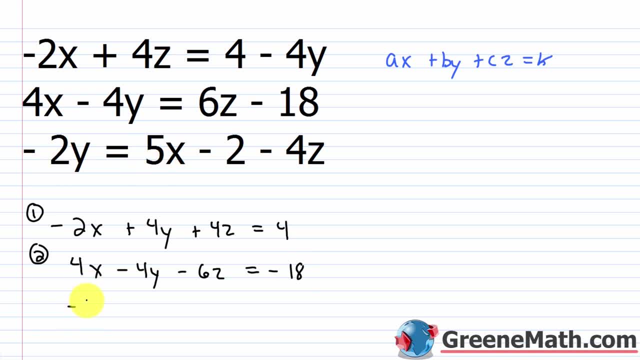 For the next guy, let's subtract five x away from each side. Let's have negative two y. next, Then let's add four z to each side. This will be equal to negative two. Let's call this equation two. Let's call this equation three. 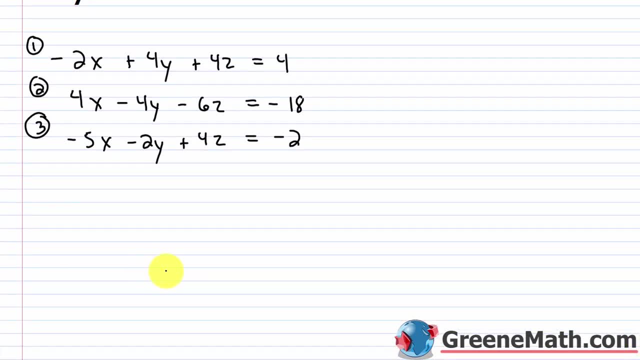 All right, So let's take a look at what we can do here. So I want to start with any two equations and I want to eliminate one of the variables. So it looks like it'd be really easy to eliminate y if I worked with equation one. 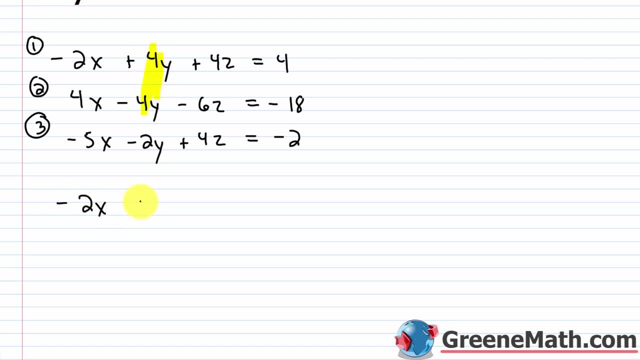 and two. So if I have negative two x plus four, y plus four, z equals four. then I have four x minus four, y minus six z equals negative 18.. What do we have here? If I add the left sides, set this equal to the sum of the right sides. 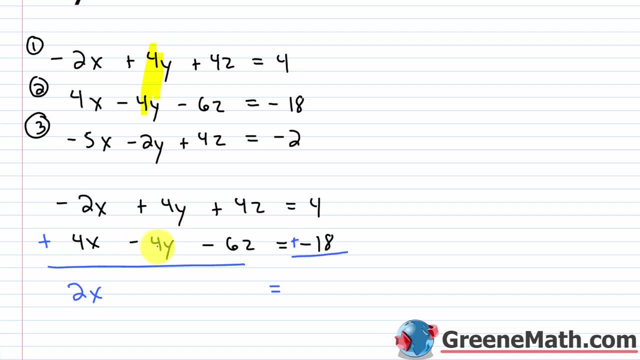 Negative. two x plus four, x is two x. Four y minus four, y is zero, That's eliminated. Four z minus six, z is minus two z. This equals four minus 18, which is negative 14.. So let's say equation four here is two x minus two z equals negative 14.. 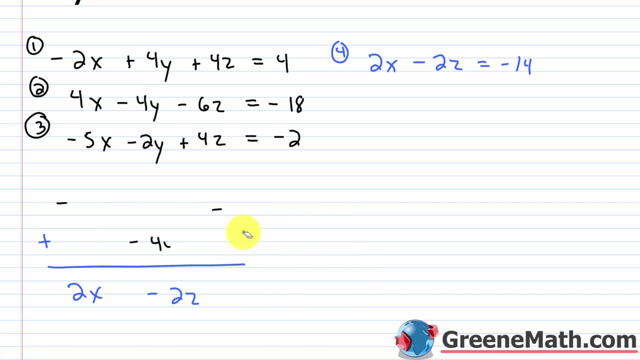 Now I'm going to eliminate the same variable, which is y, from any two other equations, So let's go ahead and use equation one and three So negative. two x plus four, y plus four, z equals four. Equation three is negative. five x minus two, y plus four z equals negative two. 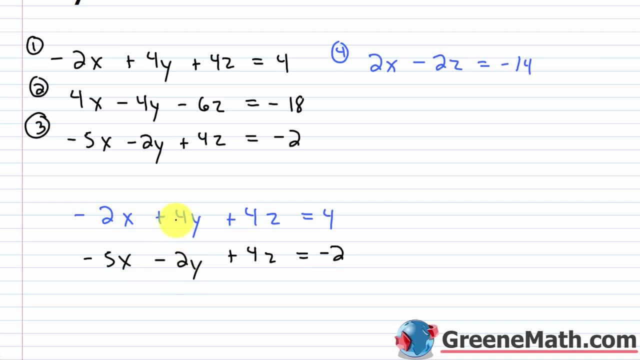 So I don't quite have what I need. If this was negative four, I'd be good to go. So I can accomplish that by multiplying both sides of the equation. two Two times negative five x is negative ten x. Two times negative two. y is minus four y. 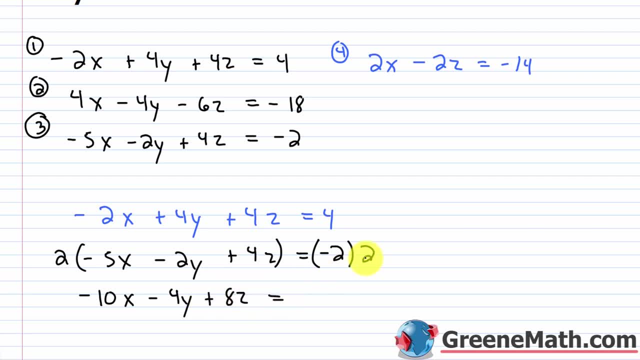 Two times four. z is plus eight z. This equals two times negative two is negative four. All right, So now let's sum the left sides. Set this equal to the sum of the right sides. Negative two x minus ten. x is negative twelve x. 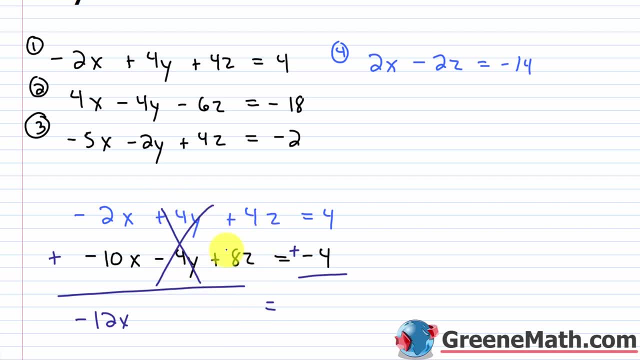 Four y minus four y is zero. Y is eliminated. Four z plus eight z is plus twelve z. And then four minus four is zero. So as equation five goes, you would have negative twelve x plus twelve z equals zero. So it looks like a pretty easy to use substitution here. 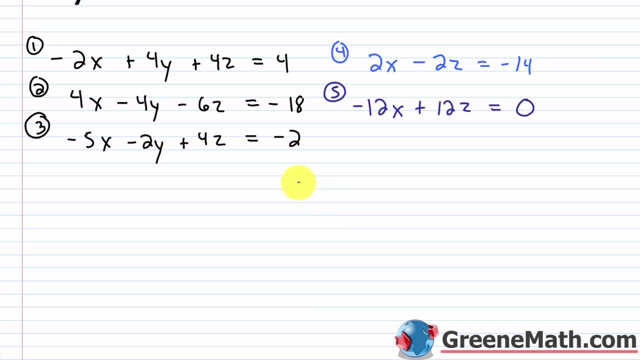 Let me take equation four and solve it for x. So I have two x minus two z equals negative fourteen. If I want to solve this for x, let me add two z to both sides of the equation. That's going to cancel. We'll have two x is equal to two z minus fourteen. 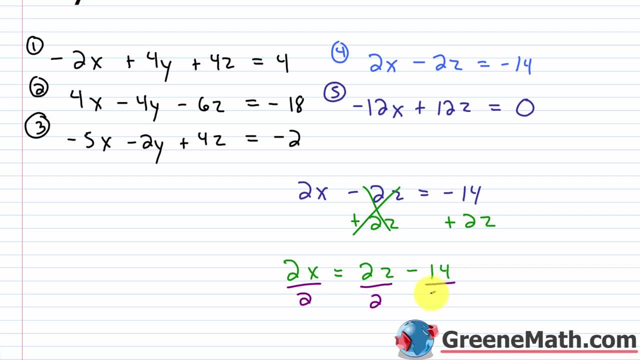 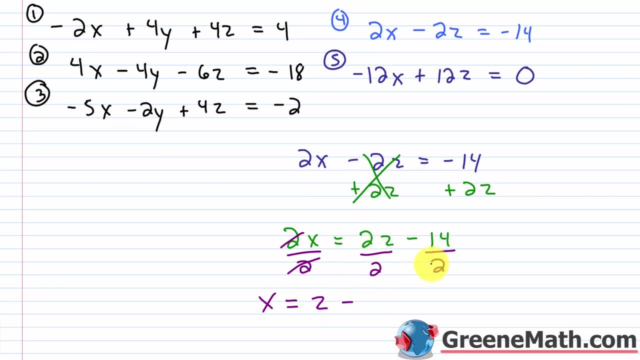 Let's go ahead and divide both sides of the equation by two. That'll cancel. We'll have: x is equal to two over two is one, So it's just z minus fourteen over two is seven. So we can say that this relates to this. 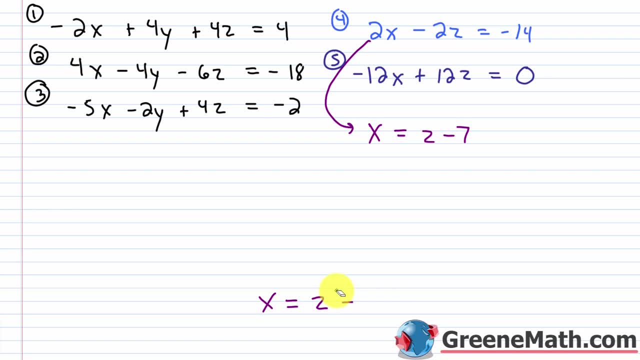 We have: x is equal to z minus seven. Now I'm just going to plug in four x in equation five, So we would have negative twelve times. plug in a z minus seven for x plus twelve. z equals zero Negative twelve times z is negative twelve z. 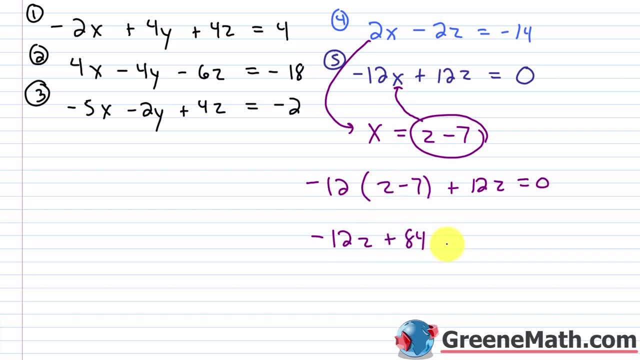 Negative twelve times negative, seven is positive. eighty four Then plus twelve z equals zero. So I want you to notice something: You have negative twelve z and you have positive twelve z. Those are going to cancel. I'm left with eighty four equals zero. 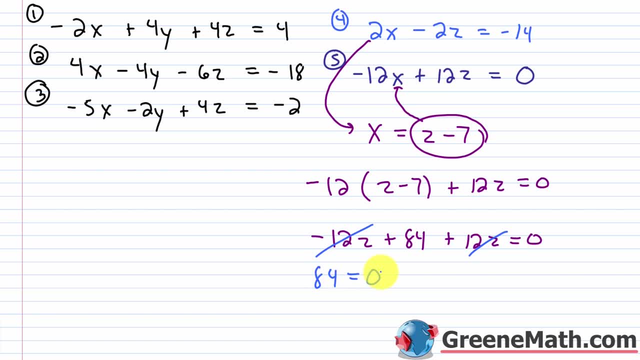 We've seen this before, Remember: your variable drops out. you've got nonsense. That means no solution. It's the same thing when you're working with a linear system with three variables. So there's no solution here. No solution, All right. so we put the symbol for the null or empty set. 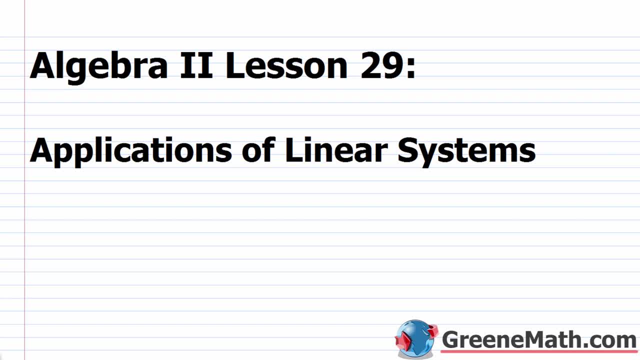 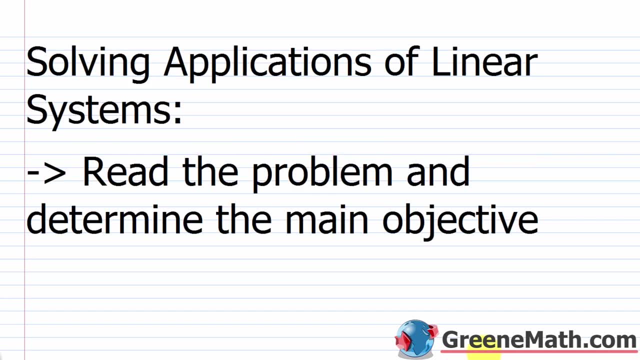 Hello and welcome to Algebra 2, Lesson 29.. In this video, we're going to learn about applications of linear systems. So throughout your study of algebra- and I mean algebra one, algebra two, college algebra, whatever level of algebra you're in- 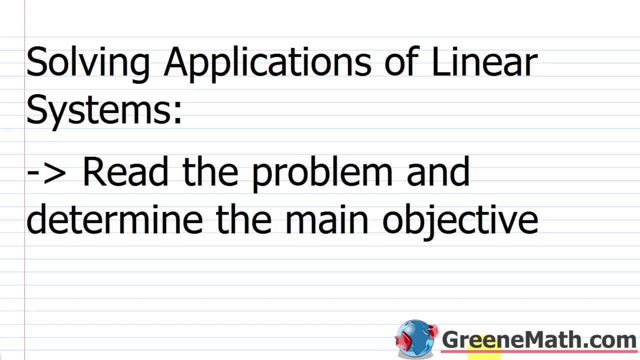 You're going to consistently run into word problems and for whatever section you're dealing with, they're generally a little bit more challenging than if you just had a problem presented to you. The reason for this is you have to dig through the information and then generate the problem and then solve it and go back. 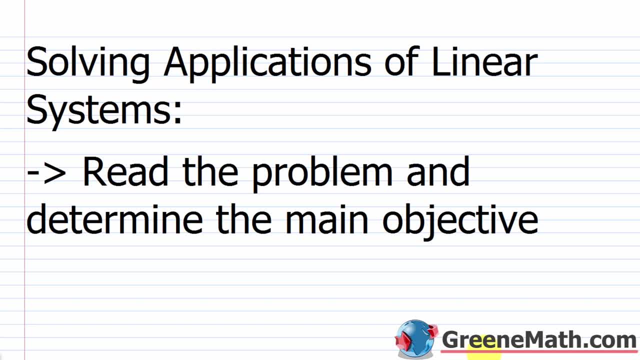 and answer and figure out if it makes sense. So in a lot of cases it will help you substantially If you have just a little procedure, a little guideline to refer to when you're working through these problems. So I'm going to give you one here and you 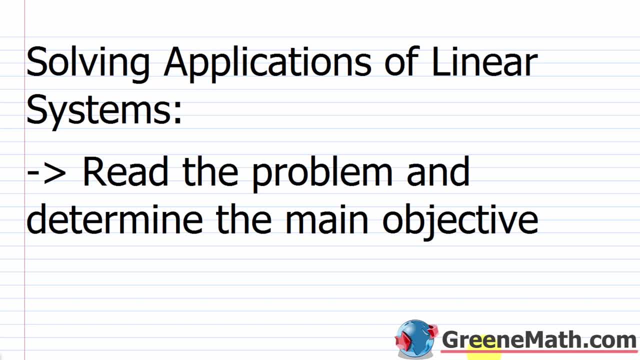 can make up your own and you can modify this whatever suits your needs. So I have here solving applications of linear systems. So the first thing, and probably the most important thing: when you're working, any word problem, I don't care what it is. 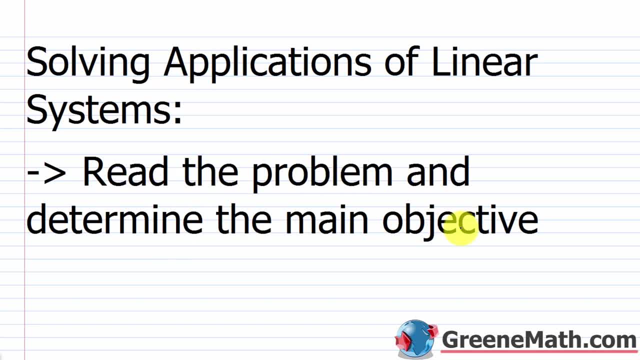 You want to read the problem and determine the main objective. If you don't know what you're being asked to find, then how can you find it Right? So that's the most important thing, All right. The next thing is to assign a variable to represent each unknown. 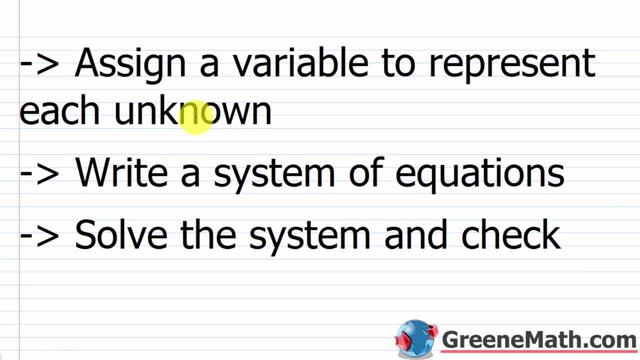 Now this changed a little bit versus when we talked about solving a linear equation of one variable, when we looked at word problems for that section. In that case I have one equation and one variable. If I have more than one, unknown. those problems are set up in such a way. 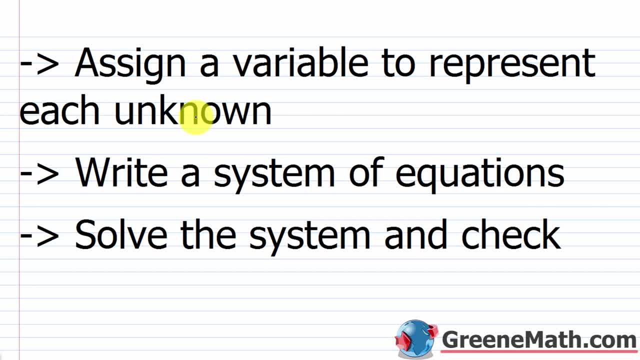 to where I can express the other unknown in terms of that first one that I said: hey, X is this, then this one is X minus this or X plus this or whatever you're given scenario is when we deal with a section on linear systems. 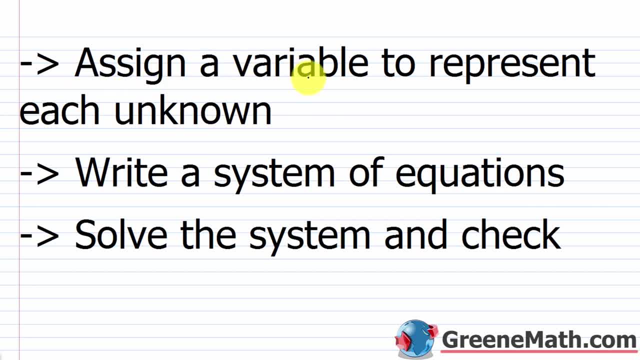 In general, the problems are set up to where you just assign a variable to represent each unknown and then you would write a system of equations. Now, for every unknown I have, I have to have an equation. So if I have two unknowns, I need two equations. 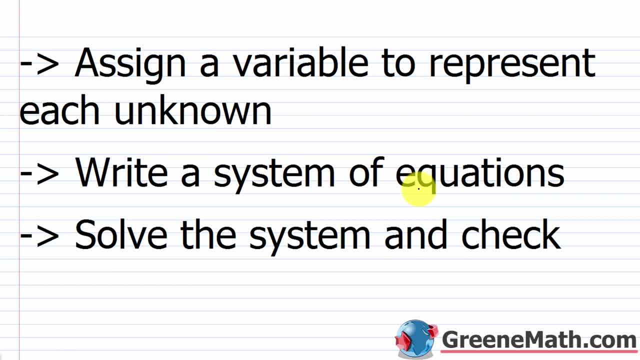 If I have three unknowns, I need three equations. If I had seven unknowns, I would need seven equations, So on and so forth. Now, once I've gone through and I've written my system of equations, I would simply solve the system. and I want to check now with word problems. 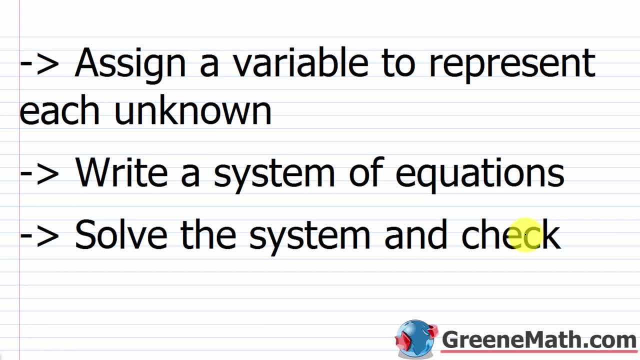 You got to make sure that when you check your answer it's reasonable. OK, if I'm on a train and it says how many passengers were on this train with me, it can't be negative seven and it doesn't make sense If I'm calculating a rate. 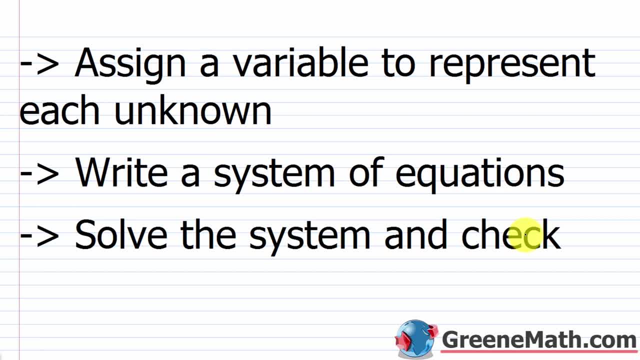 of eight. it can't be negative 30. OK, that doesn't make sense. If I'm calculating the amount of distance that was driven and it says negative two point six, that doesn't make sense. So make sure that your answer is reasonable in terms of the problem. 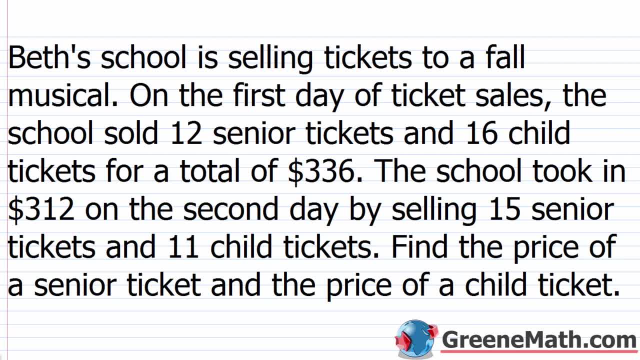 All right. So let's take a look at the first example. So we have that Beth's school is selling tickets to a fall musical. On the first day of ticket sales, the school sold 12 senior tickets and 16 child tickets For a total of three hundred thirty six dollars. the school took in three hundred. 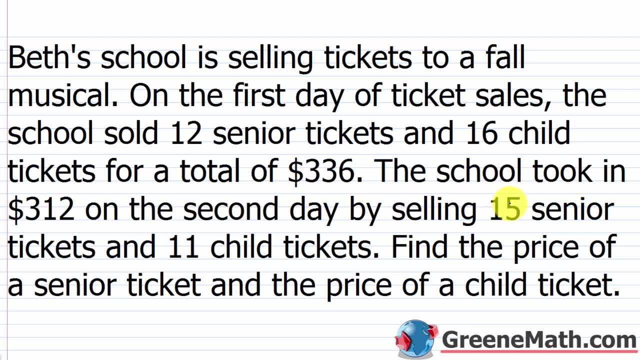 twelve dollars on the second day by selling 15 senior tickets and 11 child tickets, Find the price of a senior ticket and the price of a child ticket. So it's very straightforward here what we need to do. We want to find the price of a senior ticket and the price of a child ticket. 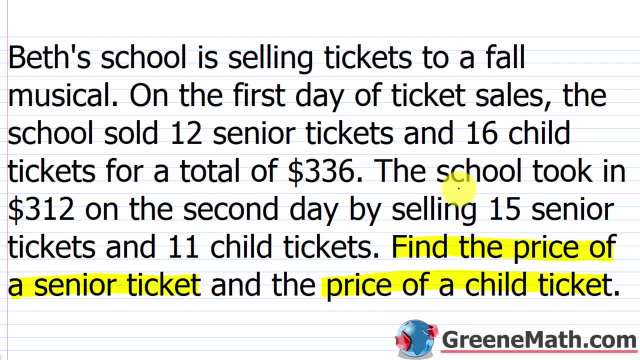 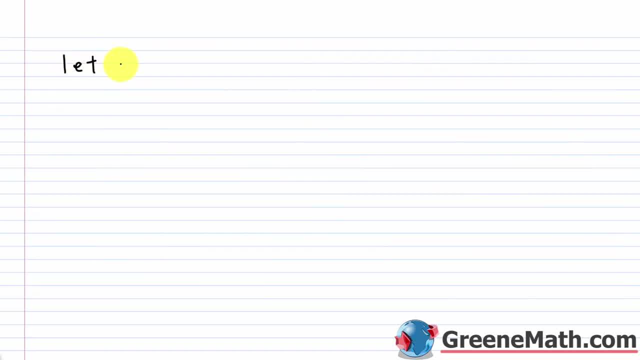 So we find the two things that we don't know, And for each unknown we represent with a variable, Let's go down to the next page, So we will let X be equal to the price Of each child ticket, And then Y. 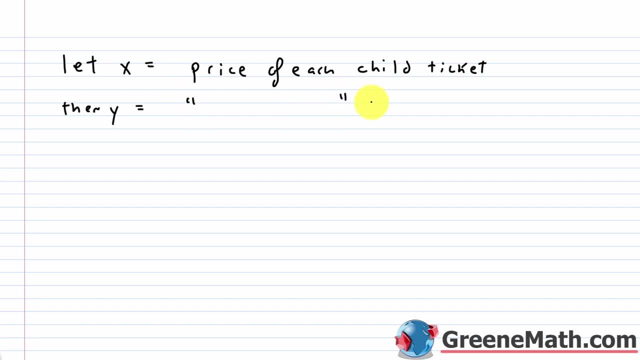 will be equal to the price of each senior ticket. All right, so now we want to go ahead and write a system of equations, So let's go back through our little problem. We're going to read and gather some information that we can use to set up a system. 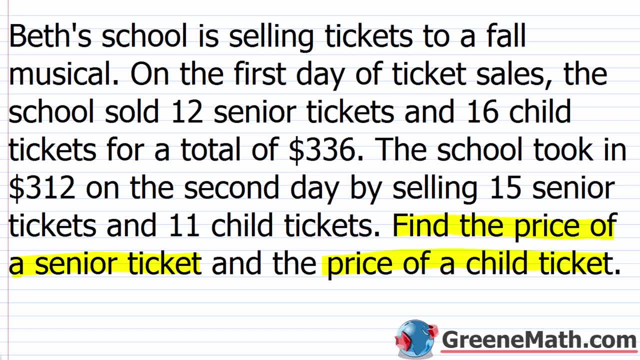 So, with these problems, they're going to give you information to build your system With this one. it tells you about ticket sales. So on the first day of ticket sales, the school sold 12 senior tickets and 16 child tickets, for a total of $336.. 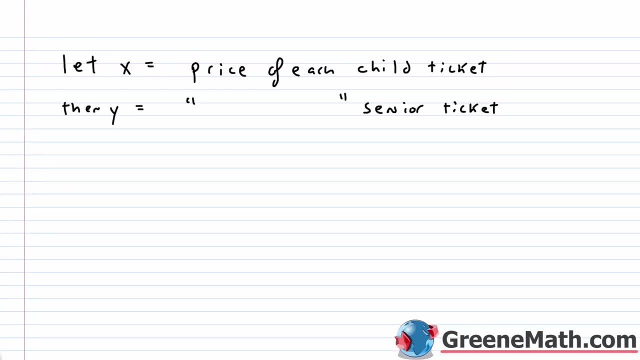 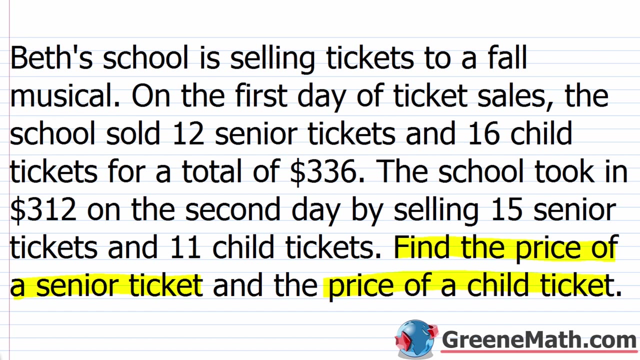 So let me go to the next page. So there was 12 senior and 16 child and it was $336.. Let's just save that information there. Let's go back Now the other scenario they give us. it says the school took in $312 on the second day by selling 15 senior tickets. 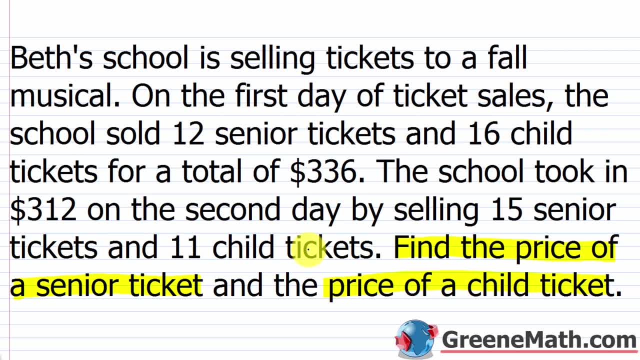 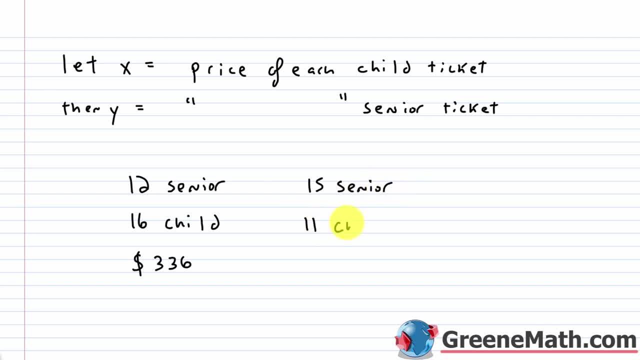 and 11 child tickets. So let's go back. So now we have 15 senior, We have 11 child And the total from this day was $312.. So I have two scenarios and this is going to be enough for me to build a system of equations. 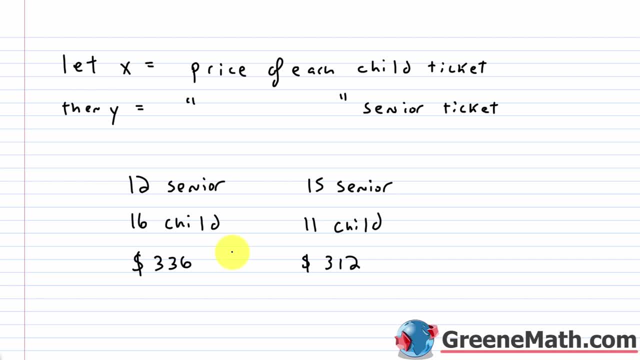 So X is the price of each child ticket. Now, if I sold 16 child tickets and X is the price of each child ticket, so let's say X with 10.. I'm not saying it is, but let's say it was. 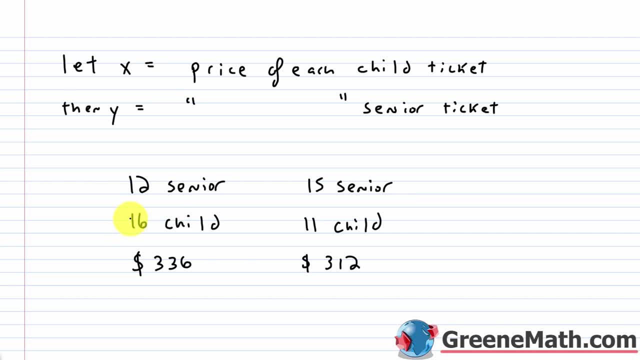 Well, 16 times 10 will be 160. So I'm going to multiply 16 times X to get the total revenue from selling child tickets that day. So in the first scenario I will have 16 times X. Then I'm going to do the same thing for senior tickets. 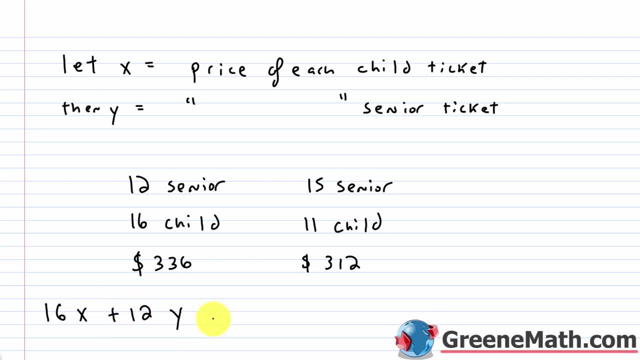 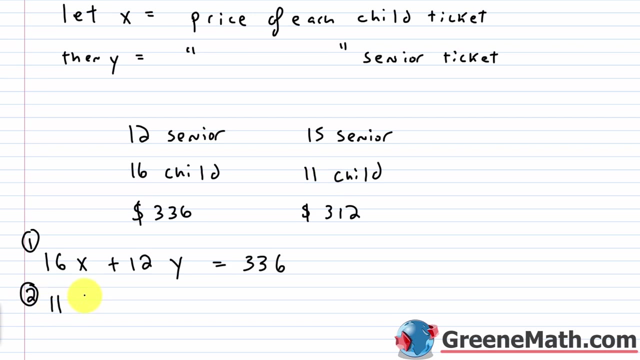 So plus 12 times Y, And this is equal to $336.. So this is my first scenario. My second scenario over here I'm going to mirror that. It's going to give me my second equation. So for child tickets, it's 11 that we sold times X dollars a piece. 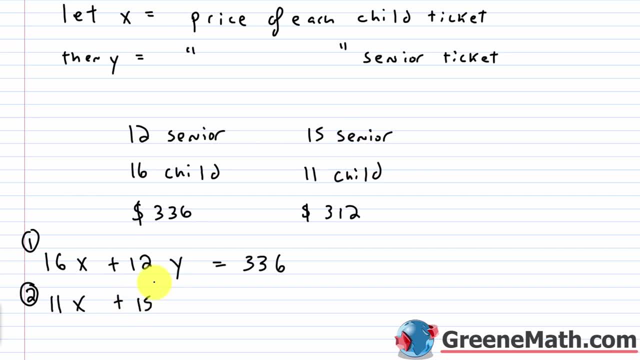 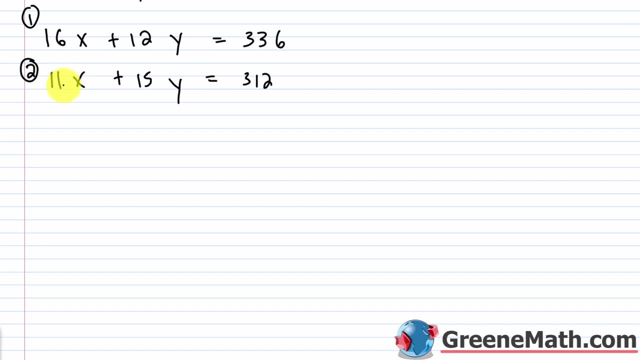 Plus for senior tickets, it's 15 sold times, Y dollars a piece, And this equals 312.. All right, So let's go through this real quick, just so everybody understands what's going on. This 16, this number here and this 11 here. 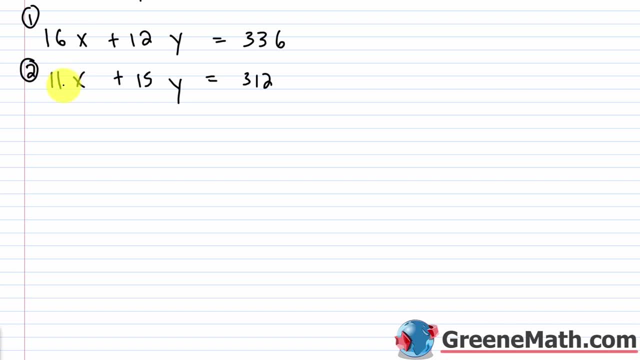 That's how many we sold, So that's a quantity. The X represents the price per ticket. So if I have the amount sold times the price each, that gives me the total revenue- in this case for child's tickets sold, Then I have 12 and I have 15.. 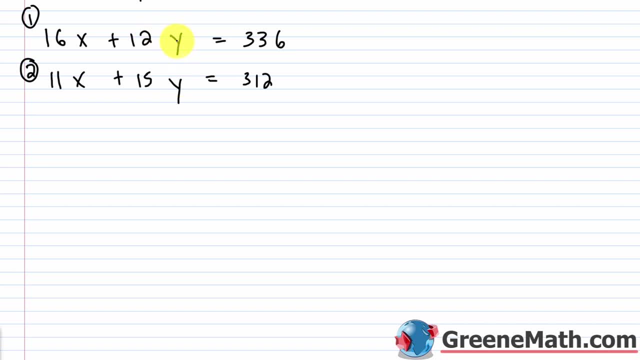 Then each one is multiplied by Y. So in this case it's 12 times Y, In this case it's 15 times Y. That's giving me the revenue for senior tickets sold. If I take the revenue from child tickets sold and the revenue from senior tickets sold and I combine them together, 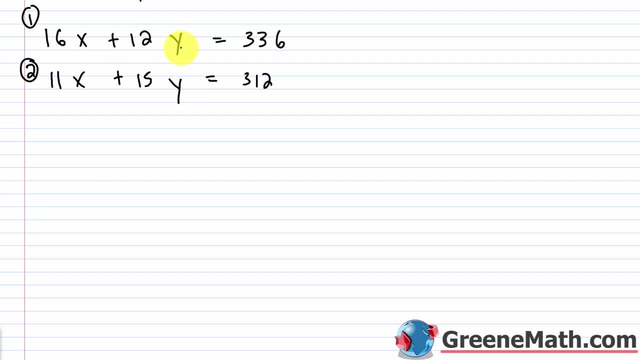 I should get the total revenue for the day. So here that total revenue was 336.. Here that total revenue was 312.. So that's how we went about setting up our system of equations, And now it's just a matter of solving the system for X and Y. 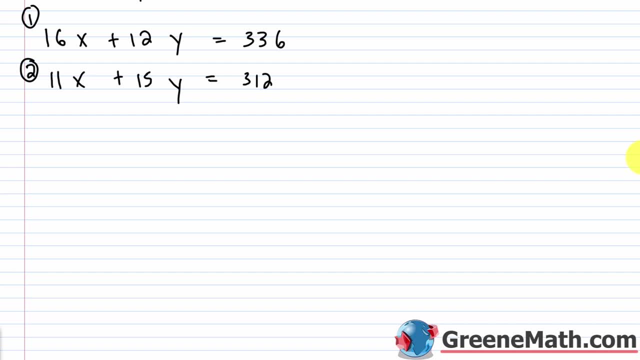 And we can report our answer. We'll know X is the amount per child's ticket sold and Y is the amount per senior tickets sold. All right, So let's go ahead. Let's use substitution. I think that'd be a little bit easier here. 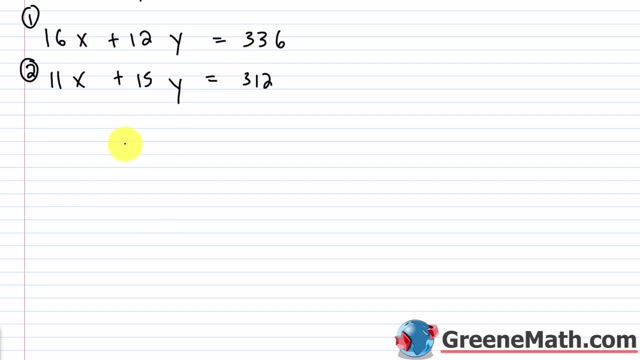 So I'm going to take equation one and I'm going to solve it for Y. So I have 16 X plus 12. Y is equal to 336.. So let's subtract 16 X away from each side of the equation. This would cancel. 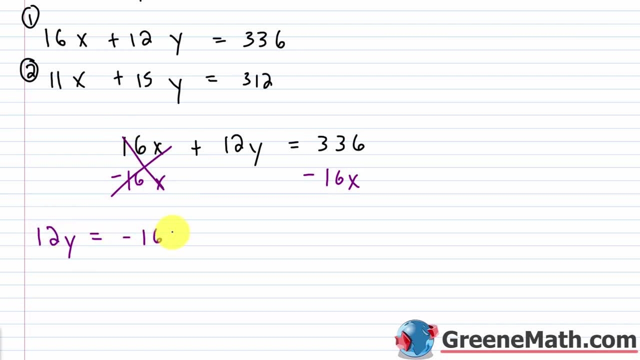 I'll have 12. Y is equal to negative 16, X plus 336.. The next thing I want to do is I want to divide both sides of the equation by 12.. So this will cancel. I'll have: Y is equal to negative 16 over 12.. 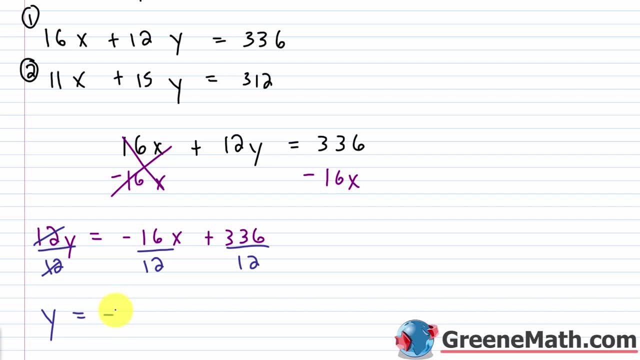 We know that's negative. 16 and 12 are each divisible by four. So if I divide 16 by four, I get four. If I divide 12 by four, I get three. So this would be negative. four thirds X, and then 336 over 12 is 28.. 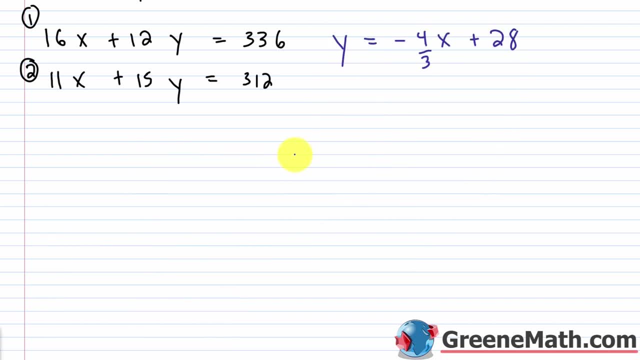 So this would be plus 28.. So I have solved equation one for Y. So now I'm going to plug in for Y in equation two. So here's Y and I'm going to plug in: Remember, Y is equal to, or Y is the same as, negative four thirds X plus 28.. 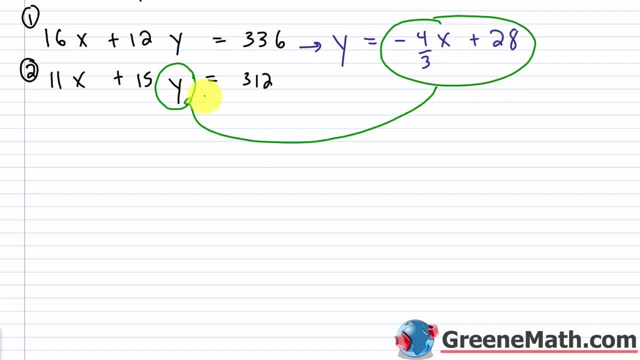 So this will get plugged in here and then I'll have a linear equation in X. I'll just have one variable, So 11, X plus 15.. I'm going to substitute in the negative four thirds X plus 28, like that quantity. 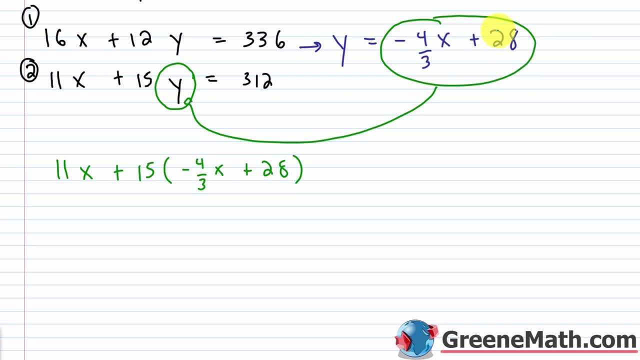 Again, make sure you use parentheses, because 15 is multiplied by this whole quantity and this equals 312.. So I will have 11 X plus. I'll do 15 times negative. four thirds X plus 15 times 28 equals 312.. Now let's deal with this. 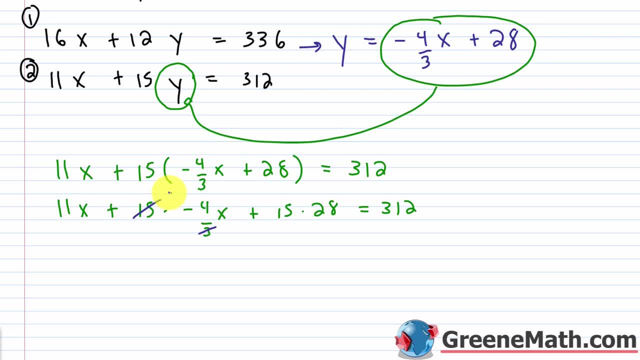 So 15 times negative, four thirds 15 would cancel with three and give me five. Five times negative. four is negative 20.. So this would be 11 X minus 20 X plus 15 times 28 is 420 and this equals 312. 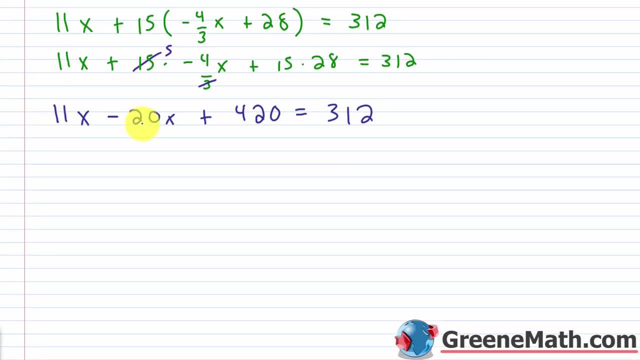 All right, let's go down and get a little bit of room going. So 11 X minus 20 X. we know that's negative nine X, So let's write negative nine X. Let's subtract 420 away from each side of the equation. 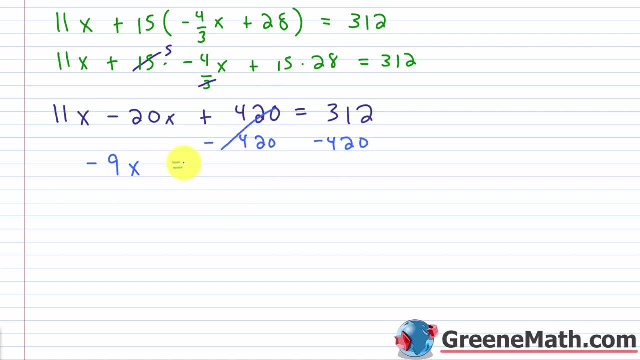 That'll cancel. So negative nine. X is going to be equal to 312 minus 420 is going to give me negative six. So let's go ahead and divide both sides of the equation by negative nine. So this will cancel with this and I'll have: X is equal to 12.. 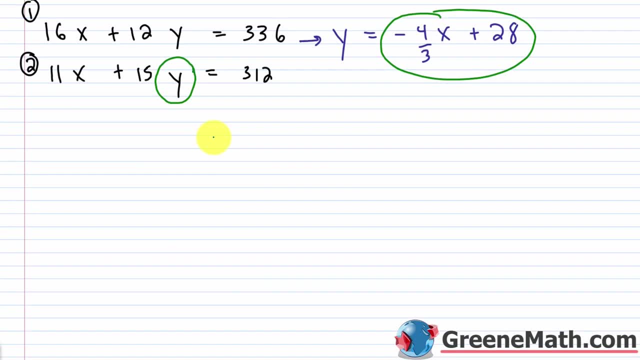 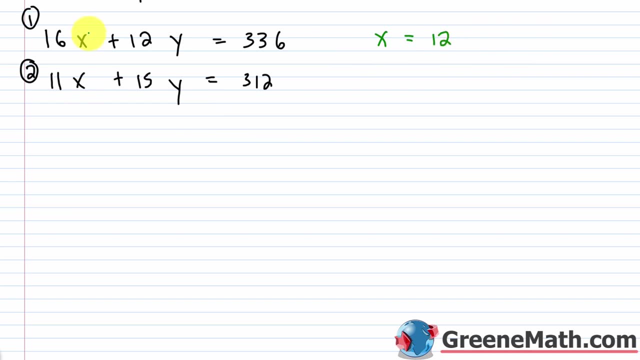 All right. so now that I know X is equal to 12, let's erase everything. Let's go back up here. I can erase this. So X is equal to 12.. So I can plug a 12 in for X, either an equation one or two. 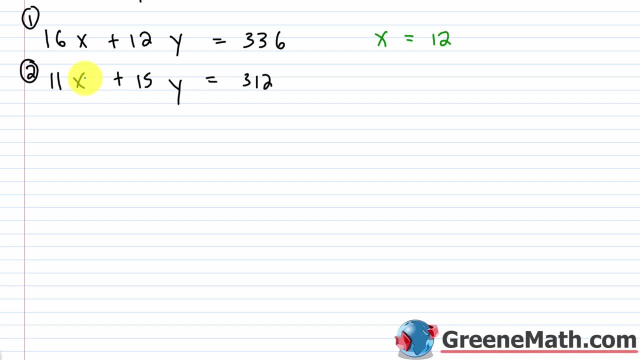 doesn't matter and solve for the unknown Y. Let's go ahead and plug in a 12 for X in equation two. So I would have 11 times 12 plus 15 Y equals 312.. 11 times 12 is 132. 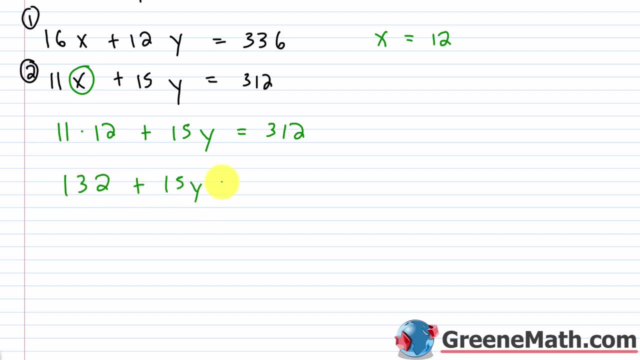 So I'd have: 132 plus 15 Y is equal to 312.. Let's subtract 132 away from each side of the equation. That's going to cancel. We'll have: 15 Y is equal to 312. minus 132 is 180.. 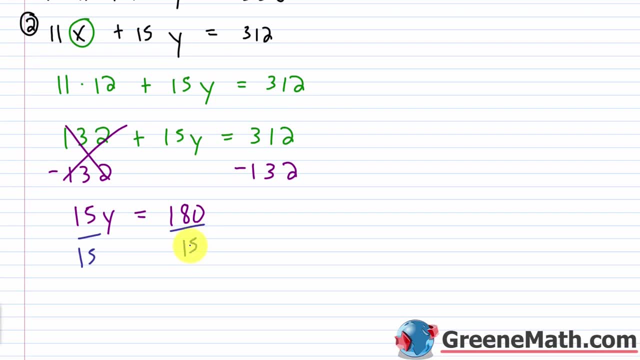 So let's go ahead and divide both sides of the equation by 15.. 15. And we'll find that Y is equal to 12. So X and Y are the same value. They're each 12.. So remember, X was the price of each child ticket. 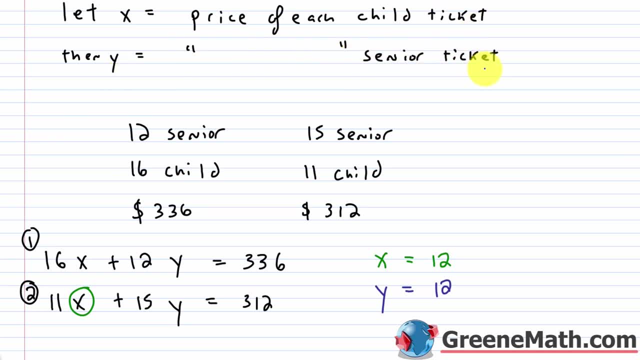 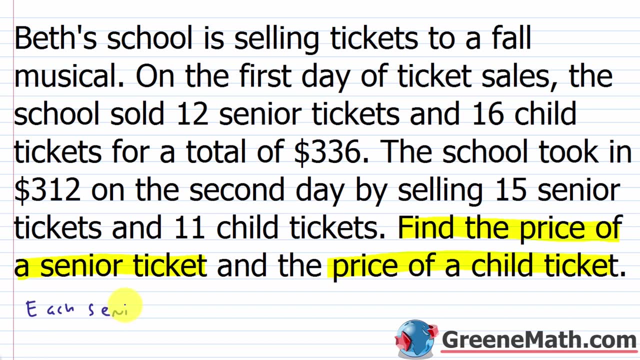 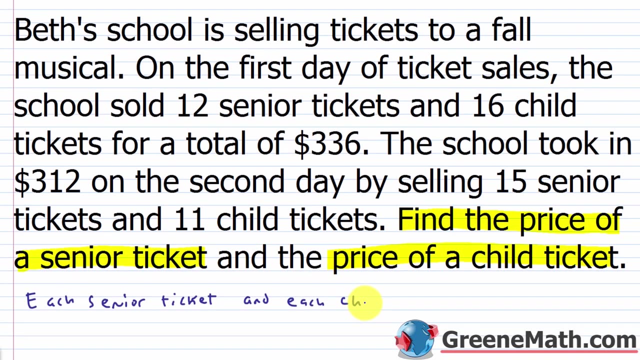 And Y was the price of each senior ticket. They're each 12. So we can go ahead and answer and say that each senior ticket And each child ticket Sold for $12.. Now can we verify this? Yeah, quite easily. 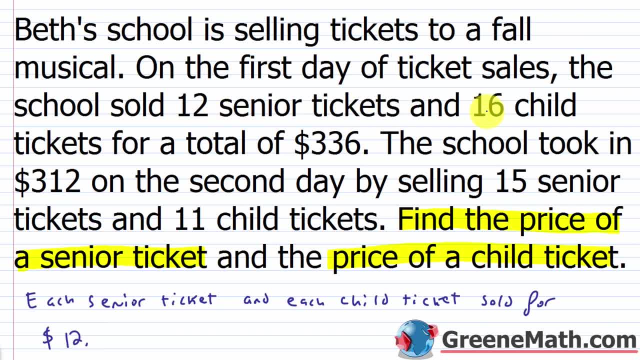 If, on the first day, we sold 12 senior tickets and 16 child tickets, Well, since the price is the same, I might as well say okay. well, I sold a total of 12 plus 16 or 28 tickets. 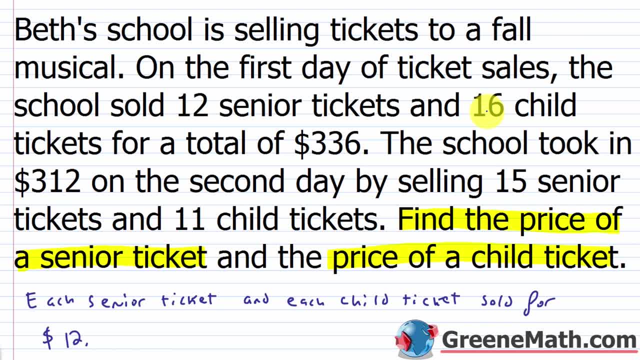 Now, if I took the 28 tickets I sold and I multiplied it by a price of $12 each, the total amount that would be received is $336.. So that one checks out. Then, in the other scenario, the school took in $312 by selling 15 senior tickets and 11 child tickets. 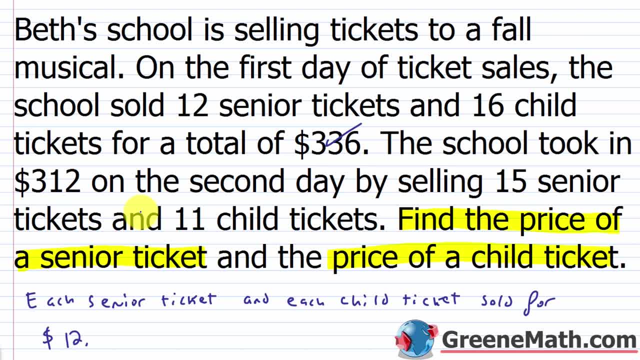 So 15 plus 11 is 26.. So 26 total tickets that day, And there again $12 a piece, because a senior ticket and a child ticket both sell for $12.. So 26 times 12 would give me 312.. 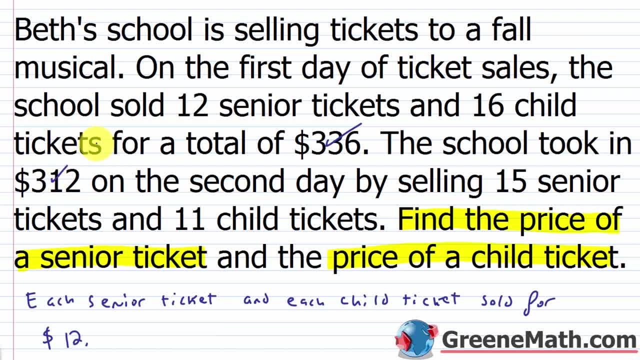 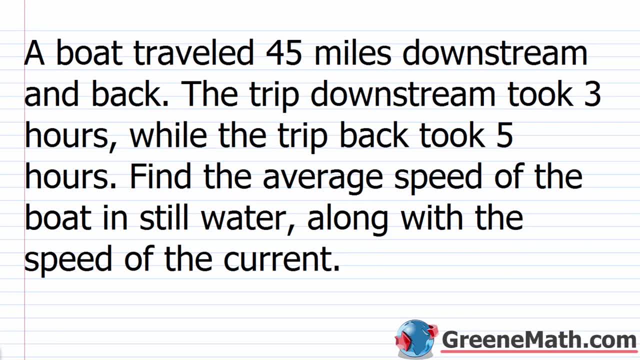 Right, So they would have taken $312 in that That day. So the answer is correct here. Each senior ticket and each child ticket sold for $12.. All right, So for the next problem. a boat traveled 45 miles downstream and back. 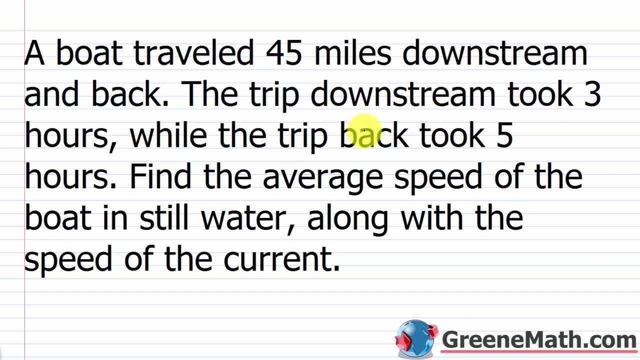 The trip downstream took three hours, while the trip back took five hours. Find the average speed of the boat in still water, along with the speed of the current. So what do we need to focus on here? Well, there's two things. we want to find the average speed. 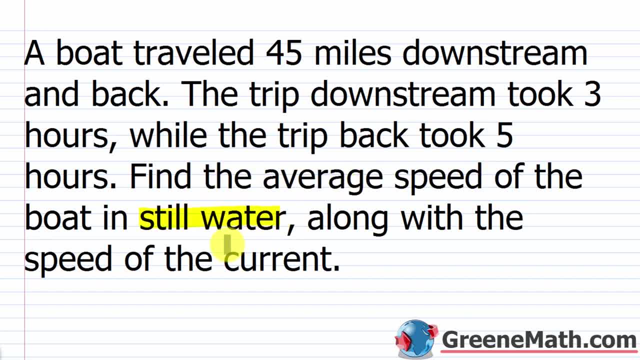 of the boat in still water, meaning if there was no current, how fast would the boat go, and then also the speed of the current. So we would start by just assigning a variable to each of those, So a variable to the speed of the boat in still water and to the speed of the current. 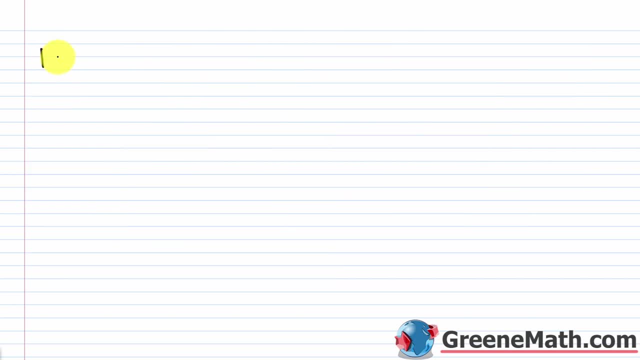 So let's go down. Let's let X be equal to the speed of the boat, And this is in miles per hour in still water. OK, then Y would be equal to the speed of the current. so the speed of the current. 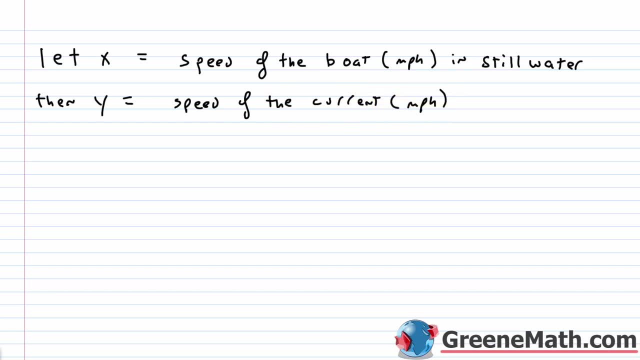 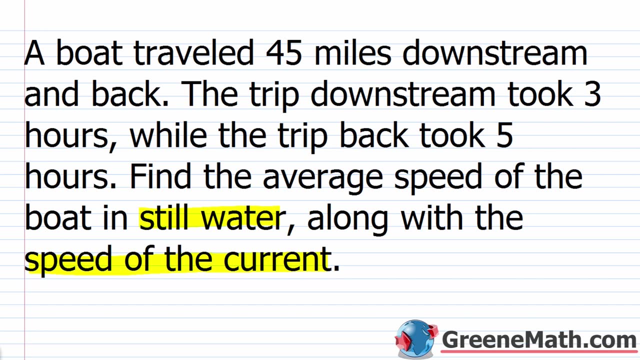 Again, this is in miles per hour. Now let's go back Now in order to answer these two questions. we want to think a little bit about what's going on here. So the boat traveled 45 miles downstream and back. 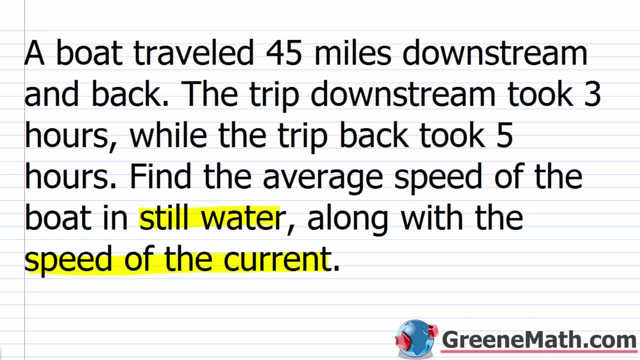 Downstream means you're going with the current. If you're going with the current, you're going to go faster. Just think about taking like an inflatable raft and just putting it in the water and going with the current, even though you don't have a motor or some kind of propeller to move you. 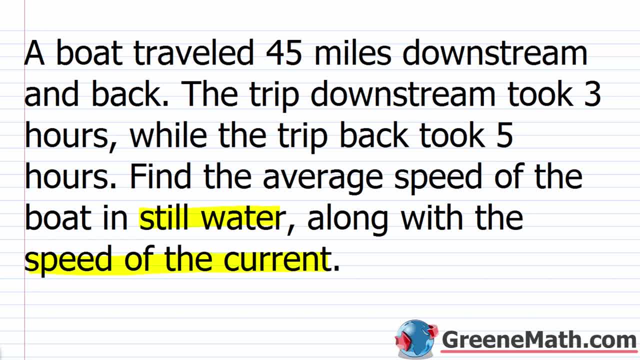 You're being moved by the current, So the current has a general speed that it's going to push you at. Now, if you're going upstream, you're fighting the current. You know, have you ever been in a rowboat or anything, or even a simple boat? and 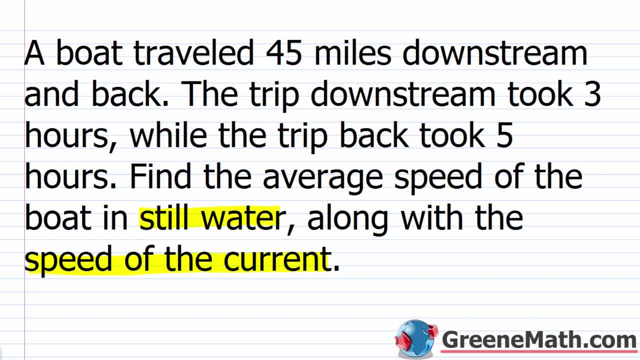 you're trying to fight the current, you know it's very hard because you're dealing with a force that's pushing against you now. So the trip downstream took three hours, while the trip back, which would be upstream, took five hours. So, of course, if you're going downstream, 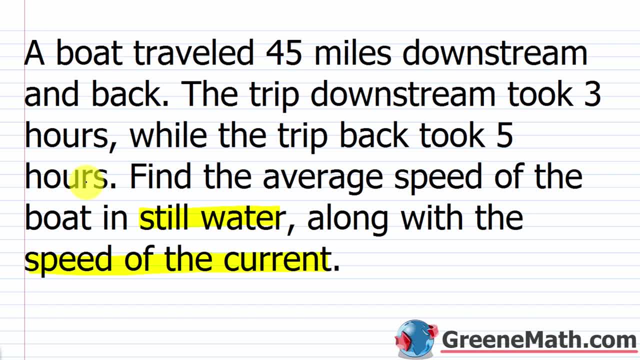 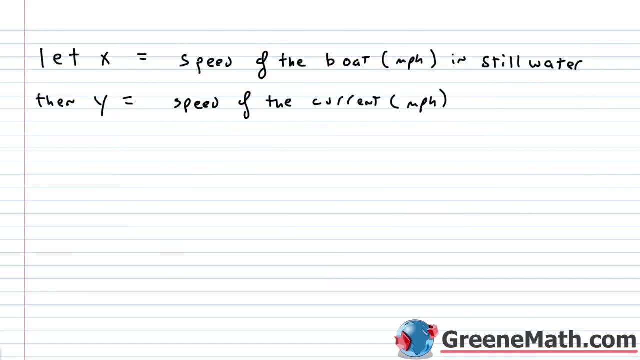 if you're going with the current, it's going to take you less time because you have a little helping hand. So, thinking about this, let's go back down. This is a motion word problem. So for a motion word problem, we think about the distance formula, right. 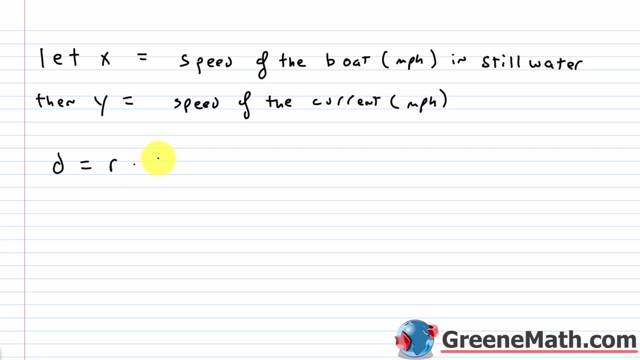 Distance is equal to the rate of speed, times, the amount of time traveled. And a lot of times when we have a motion word problem, it's usually easiest to just use a little table. So you have two scenarios. The first one would be downstream. 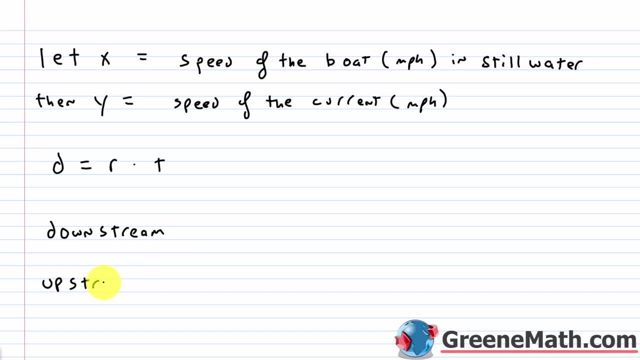 The second one would be upstream, So you have your distance and that's equal to The rate times the time. So let's see if we can fill in this information. So downstream when we're doing our trip, let's go back up. 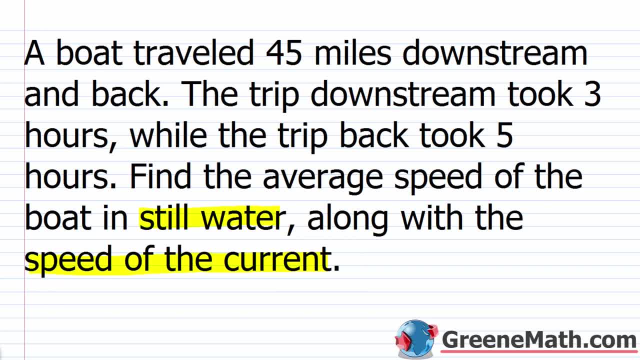 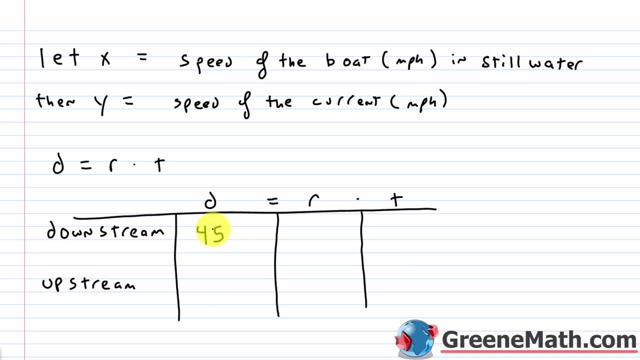 The boat traveled forty five miles, so that's the distance. So downstream and back. the trip downstream took three hours. Let's just stop there. So we're given a distance of forty five miles. We know that forty five the rate of speed we're not given. 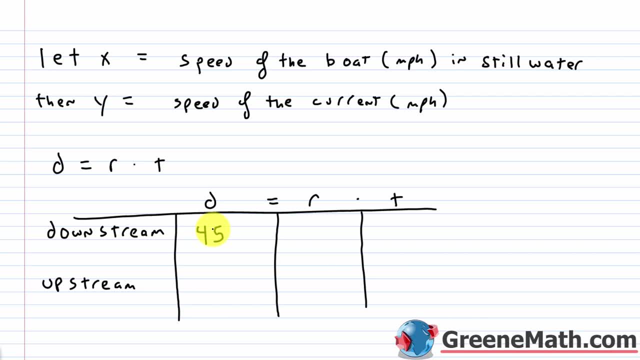 We can use our variables to work with that. But the time we are given for the trip downstream, we're told the time is three hours, So we have that. So for the rate if I'm going downstream I have the speed of the boat in still water. 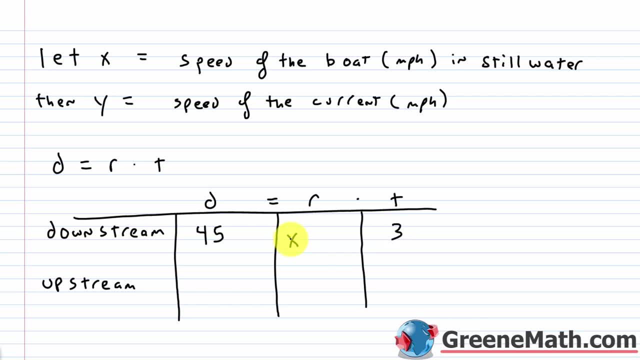 So if there was no current at all, that's X, And I also have the speed of the current. that's helping me Right. So I would increase the speed by that amount. So X plus Y, X plus Y would be my rate of speed here. 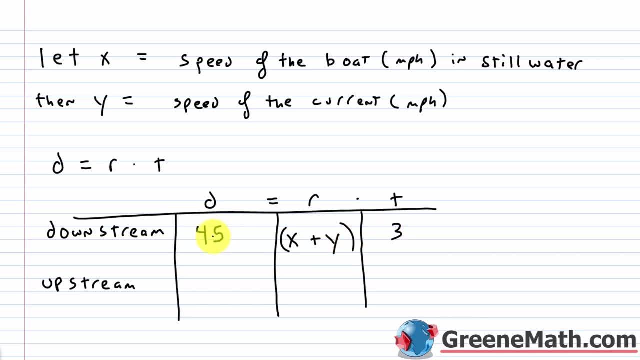 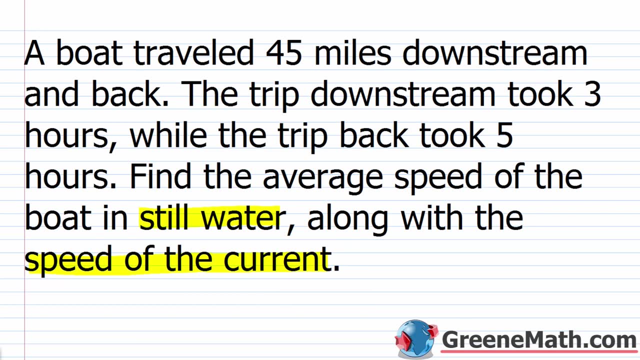 So this times, this would give me this. Now, for upstream, It tells us what. Well, the distance is the same. The only difference is the rate of speed and the time. The time now is five hours. Let's go down, So the time is five. 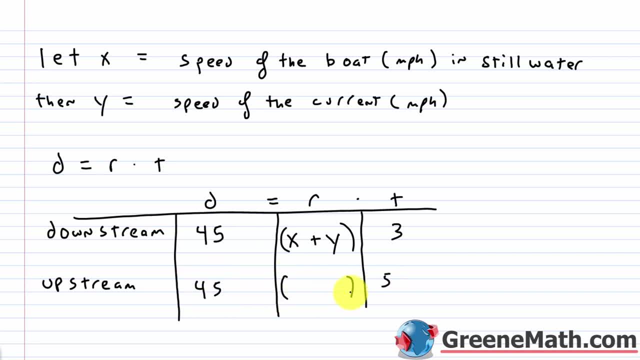 The distance is forty five, The rate of speed is going to be different. here You have the speed of the boat in still water, But since you're going upstream, you're now fighting the current, So you have to subtract away. Y. OK, you have to subtract away Y. 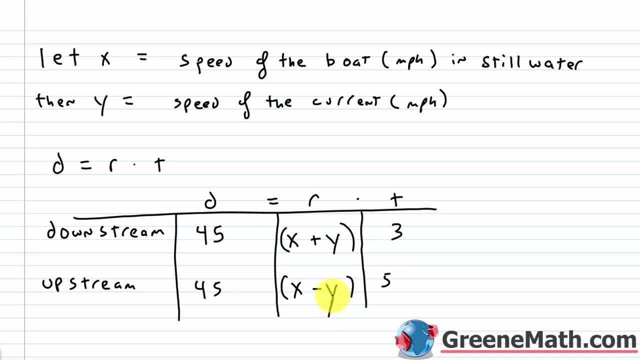 And the reason for that is your boat is fighting, You're in the still water, You have a certain speed. If you all of a sudden get put against the current, you have to subtract away the speed of that current. So, as an example, if I was going six miles an hour, 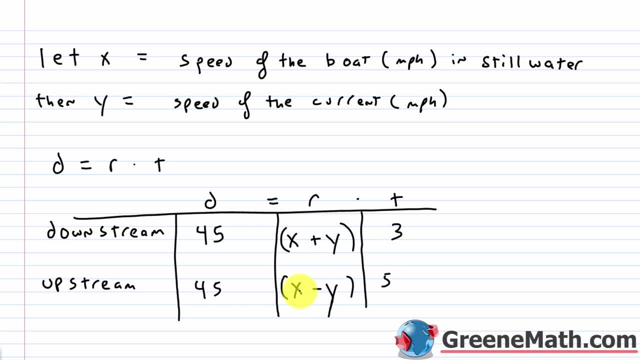 in still water and the current was three miles an hour. Well, if I'm fighting the current, then now I'm going six minus three or three miles an hour. So that's where we get this calculation here. Now I have a linear. 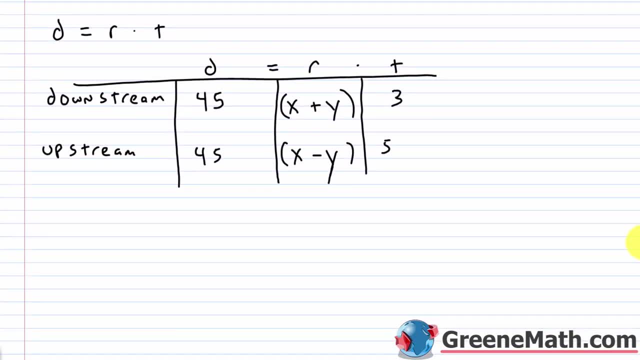 system in two variables. if I look at my little table Again, a distance is equal to a rate of speed times a time. So for downstream I have this. Let's label this equation one We have three times the quantity X plus Y is equal to forty five. 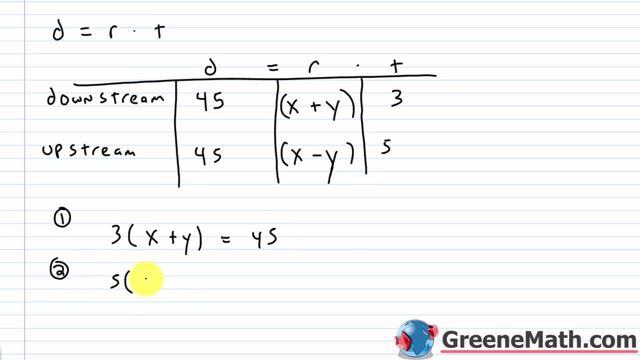 For equation two I would have five times the quantity. X minus Y is equal to forty five. Now for this system it's going to be really easy to use substitution Inside the parentheses. you see you have plus Y and minus Y. 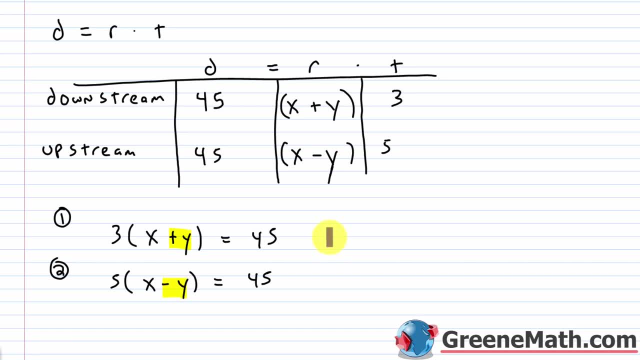 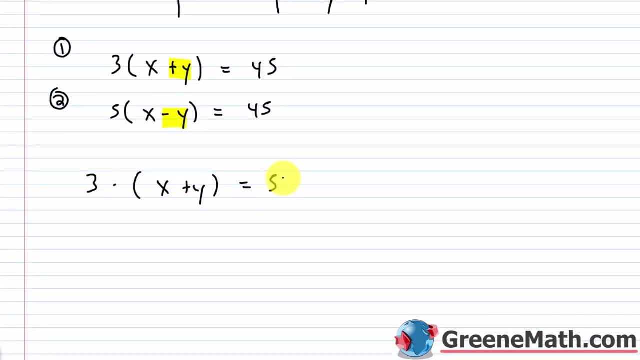 So the way we're going to do that, let me just kind of move this over here. If I have three multiplied by the quantity X plus Y, this is equal to forty five. I can divide both sides of this equation by three. Again, this is multiplication, so this would just cancel. 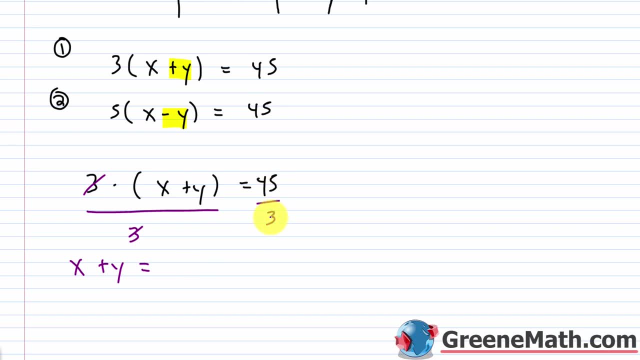 So then I'm left with: X plus Y is equal to forty. five over three is fifteen. So this I could write as: X plus Y equals fifteen. Then for this one I could do the same thing. So if I have five times the quantity, X minus Y equals forty five. 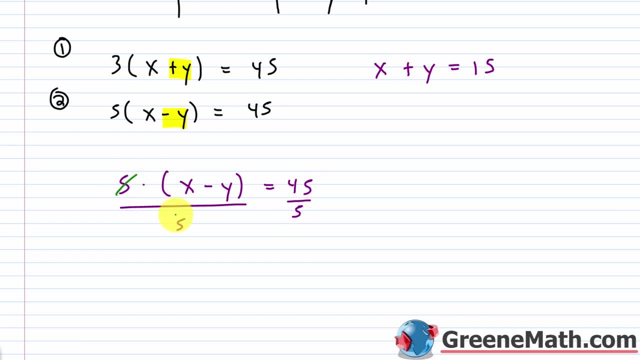 I can divide both sides of the equation by five. This will cancel. I'll have: X minus Y is equal to forty. five over five is nine. So if I add the left sides together, set that equal to the sum of the right sides. 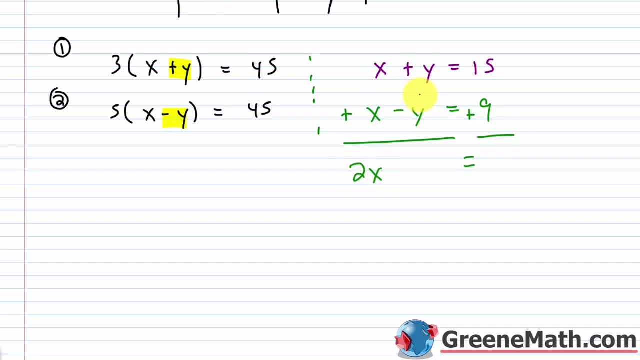 X plus X is two. X, Y plus negative Y or Y minus Y is zero. Fifteen plus nine is twenty four. So now I divide both sides of the equation by two and I get that X is equal to twelve. All right, So let's erase all this. 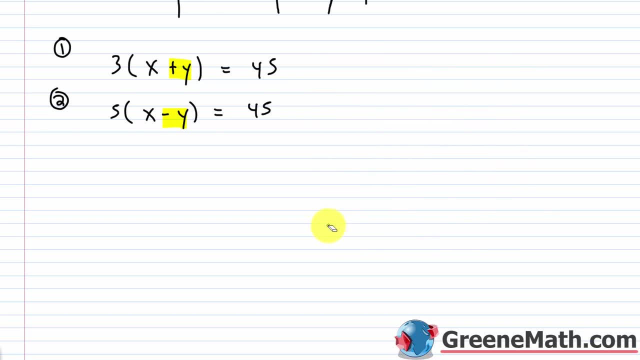 We know X equals twelve at this point. So what is Y going to be? So X equals twelve. So let's plug that back into, let's say, equation two. So we'd have five times the quantity I'd have twelve minus Y. This equals forty five. 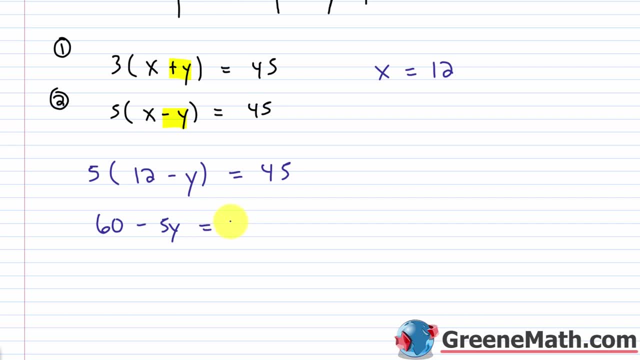 Twelve is sixty, So you'd have sixty minus five. Y is equal to forty five. We would subtract sixty away from each side of the equation. That would cancel. You'd have negative five. Y is equal to forty. five minus sixty is negative fifteen. 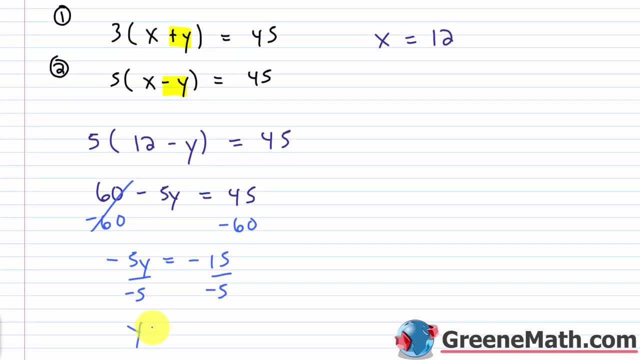 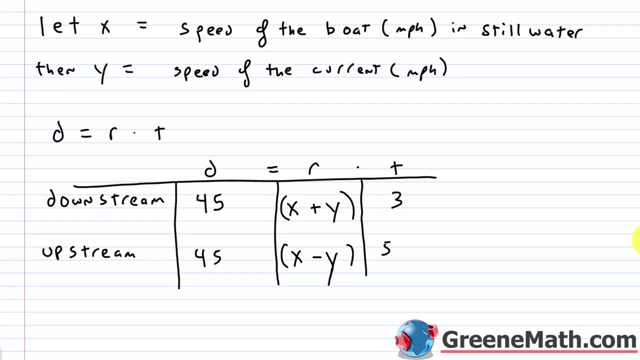 Divide both sides of the equation by negative five and you'll get: Y is equal to three. So X is twelve, Y is three. So I want you to remember that X is the speed of the boat and still water, Y is the speed of the current. 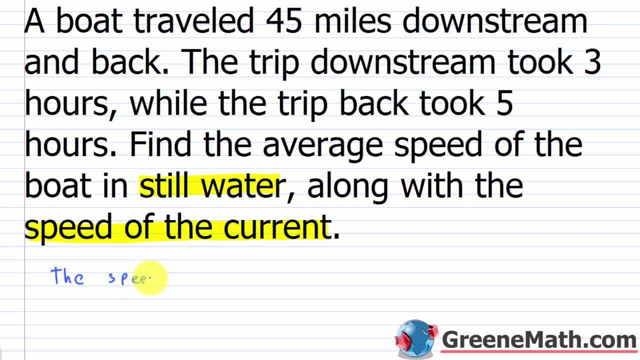 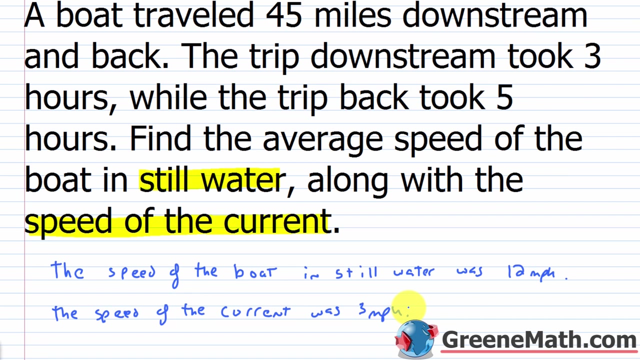 So we can say that The speed of the boat In still water Was twelve miles per hour. The speed of the current Was Three miles per hour, And we can check this pretty easily. The trip downstream took three hours. OK, so remember, distance equals rate, times time. 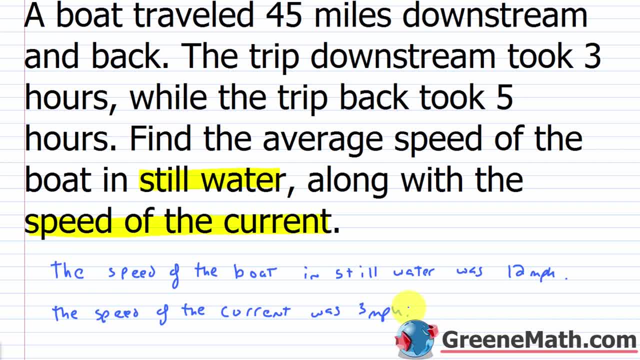 So if I'm going downstream or with the current, again, I would take my rate of speed in still water twelve miles per hour. I would add the speed of the current because it's pushing me or helping me by that much. So twelve plus three is fifteen. 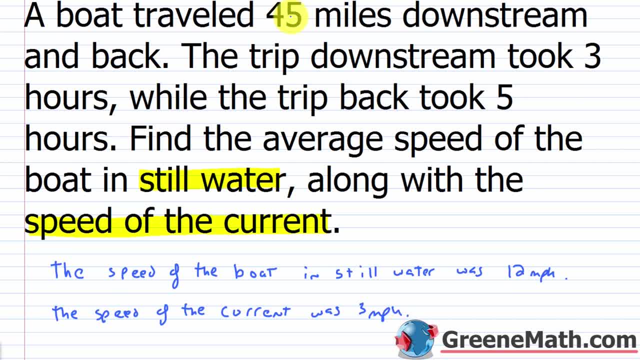 So I'm going fifteen miles an hour. for three hours That means I went forty five miles. So this one checks out. Now the trip back. we think about that. You're going twelve miles an hour in still water. Now you're fighting the current. 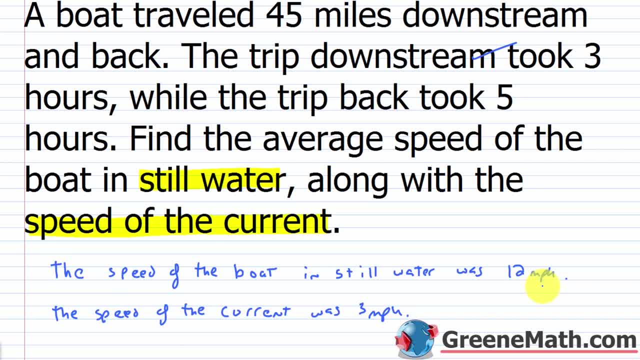 So you've got to subtract away what the current speed is. So twelve minus three is nine. So now we're going nine miles per hour for five hours. That's forty five miles, So that one checks out as well. So again, the speed of the boat in still water was twelve miles per hour. 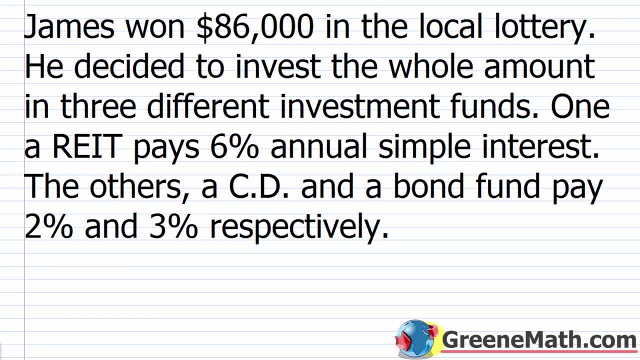 and the speed of the current was three miles per hour. Let's wrap up our lesson with one that's a little bit more tedious. So James won eighty six thousand dollars in the local lottery. He decided to invest the whole amount in three different investment funds. 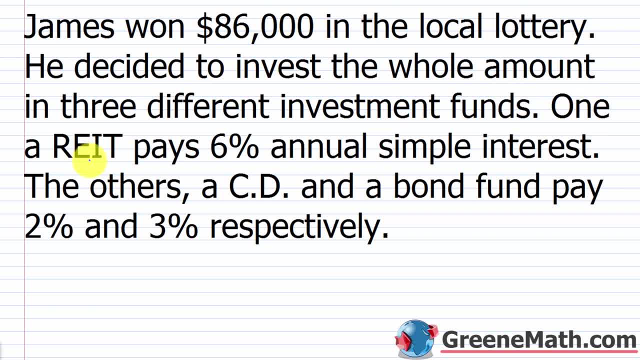 One, a REIT, which stands for Real Estate Investment Trust, pays six percent annual simple interest. So remember simple interest. you don't get interest on top of interest. So the others- a CD certificate of deposit and a bond fund- pay two percent and three. 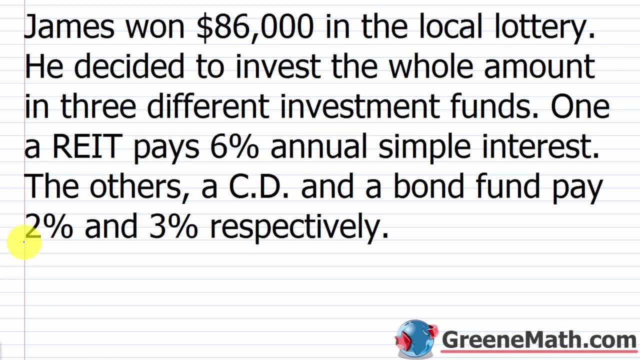 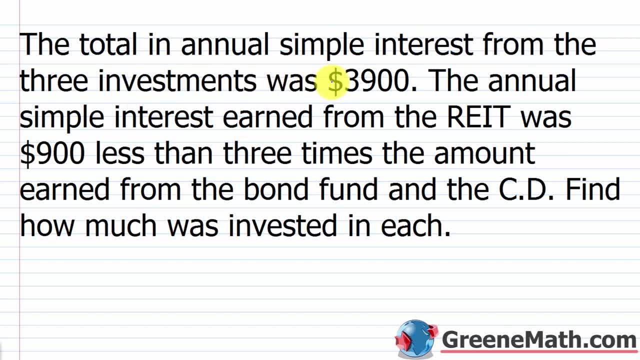 percent respectively. So that means that the CD pays two percent. The bond fund pays three percent. The total annual simple interest from the three investments was three thousand nine hundred dollars. The annual simple interest earned from the REIT was nine hundred dollars, less than three times the amount earned from the bond fund. 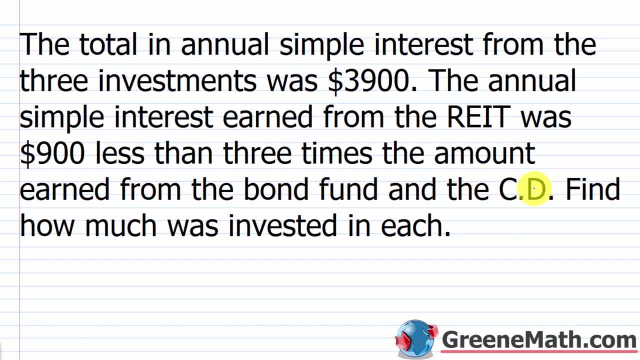 And the CD find how much was invested in each. So this is kind of a long problem with a lot of information, And when that happens you tend to get lost in the mix. I just want you to focus on one thing at a time. 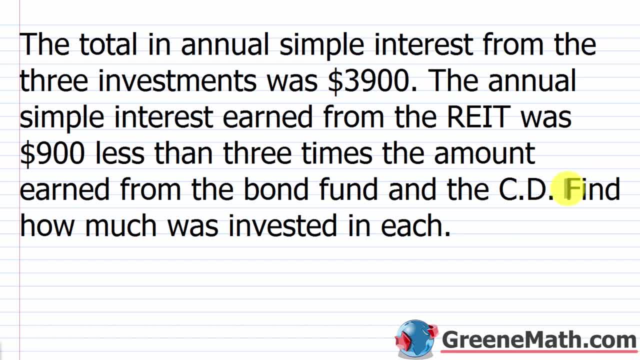 So the first thing is: what are we asked to find? We're asked to find how much was invested in each. There are three things here: There's a REIT, there's a CD and there's a bond fund, And we're not given any information. 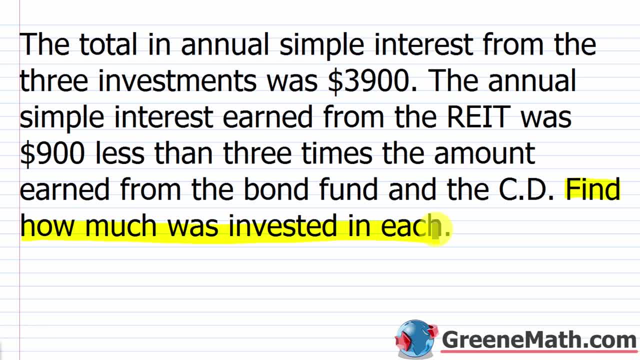 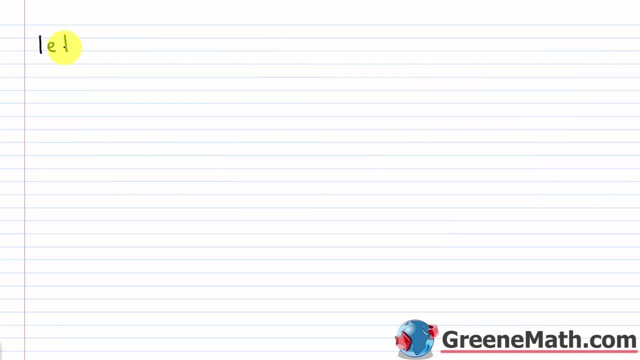 as far as how much was invested in each one. So we could use a variable to represent each amount. So we could say X, Let X be equal to the amount invested in the REIT. Again, that's a real estate investment trust. 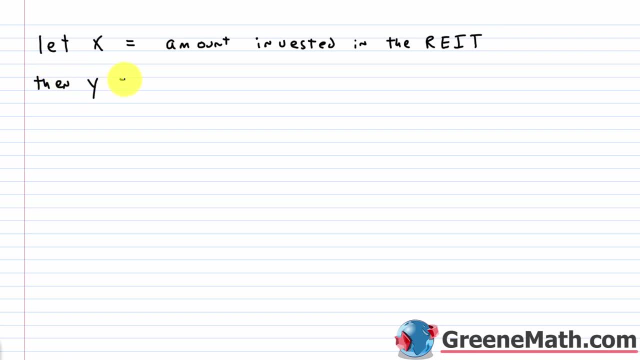 Then we could say Y Would equal the amount invested in the CD or certificate of deposit. Then we could say Z is equal to the amount invested in the bond fund. OK, so now we've represented these three amounts with variables. So we find out what X is, find out what Y is. 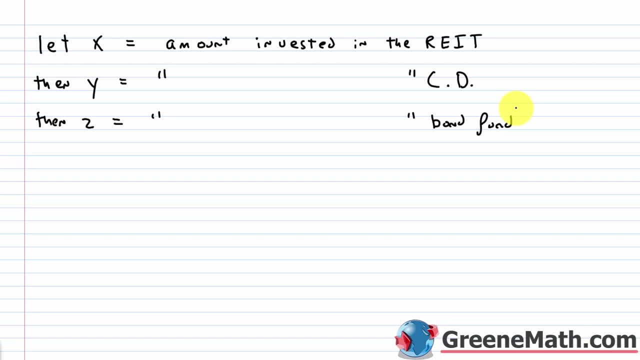 We find out what Z is and we've answered our problem. But when you have three unknowns, you need to have three equations to figure them out. OK, three unknowns, you need three equations. four unknowns, four equations, 17 unknowns, 17 equations, so on and so forth. 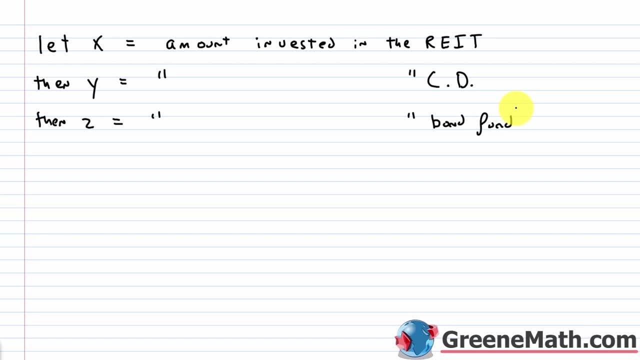 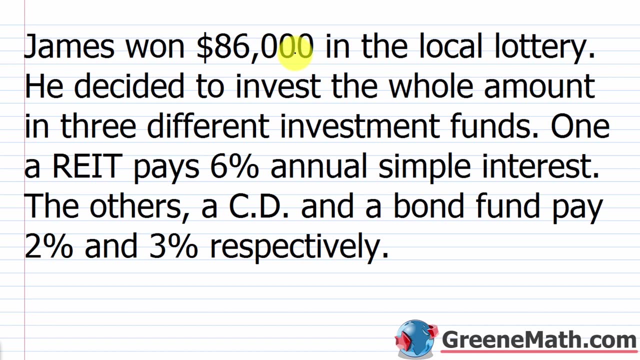 So let's go back through the problem and see if we can figure out three equations. So the first one would come from this: James won eighty six thousand dollars in the local lottery. He decided to invest the whole amount. So all of it, that's basically telling me that eighty six thousand dollars is going. 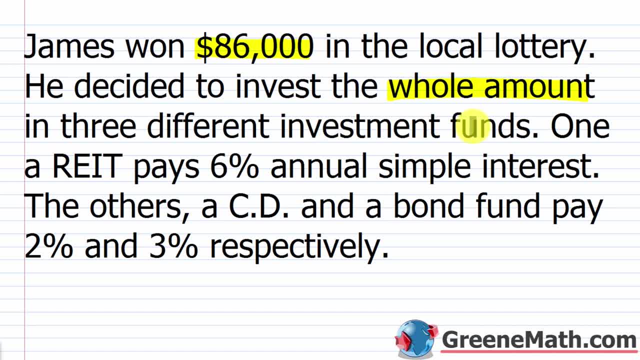 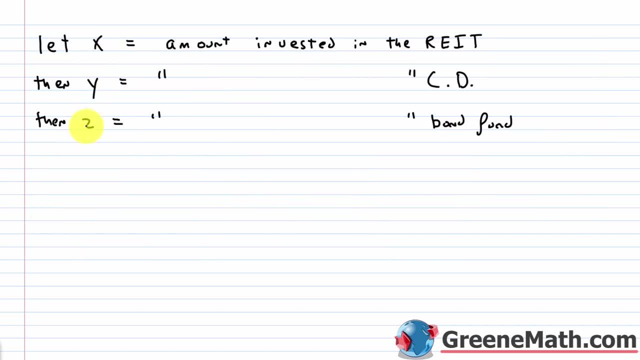 to be equal to the amount invested in the Reit and the bond fund. So we've got the Reit here and three different investment funds. So between the Reit, the CD and the bond fund there's a total of eighty six thousand dollars in them. So that tells me that if I sum X, Y and Z, 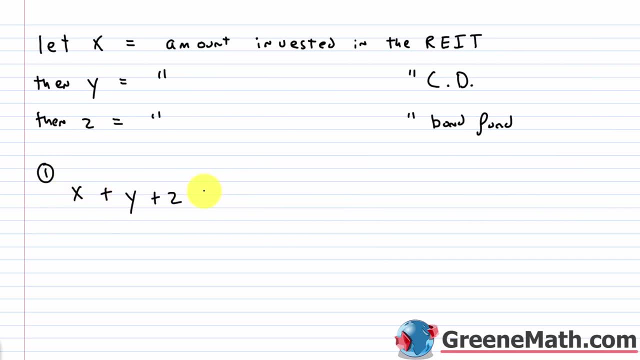 that's going to be eighty six thousand. So for equation one, X plus Y plus Z is going to be equal to eighty six thousand. And again, that's straight from the problem in the cd plus the amount invested in the bond fund, because he only puts money in those three. 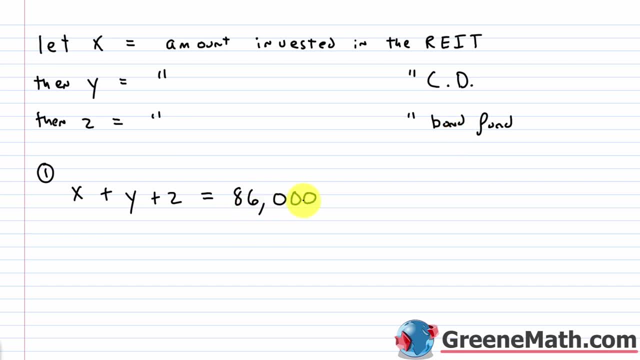 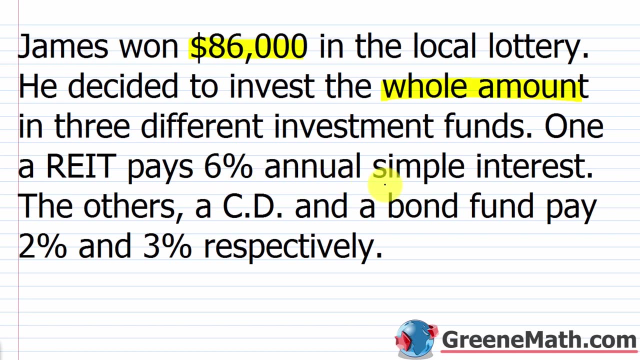 areas is going to sum to 86 000. all right, let's see if we can get another equation. all right, so the next thing we see we have a reit pays six percent annual simple interest. the others, a cd and a bond fund, pay two percent and three percent respectively. let me write that down here real fast. 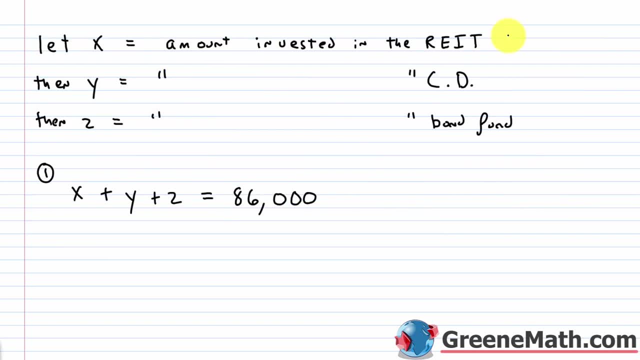 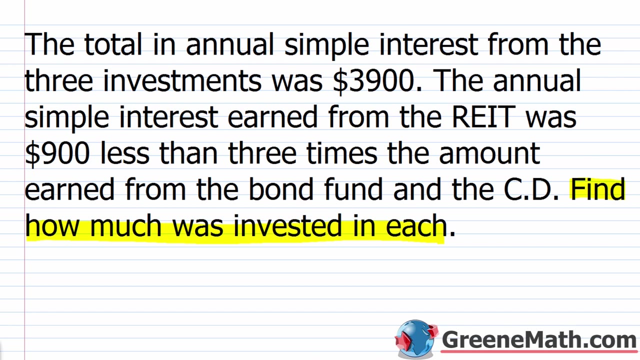 so let's put that this one pays six percent, this one pays two percent and this one pays three percent. okay, let's go back up now. the next part is where we're going to get our next equation. the total and annual simple interest from the three investments was 3 900. okay, so let's stop now. 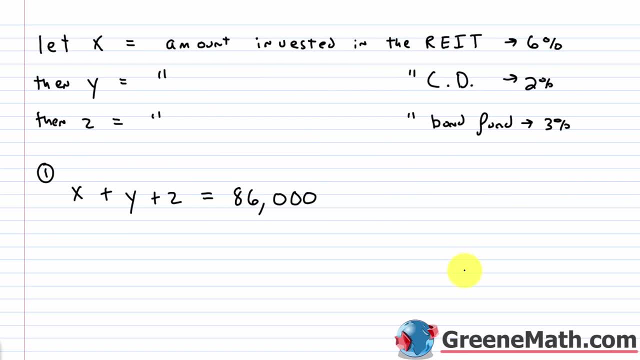 if i had one investment with simple interest interest? what is the simple interest formula? let me do this on a little sidebar over here. well, the simple interest formula, in case you don't know, it, is the simple interest earned, which is, i, is equal to the principal or amount invested, times the rate, times the time. now, in this particular case, 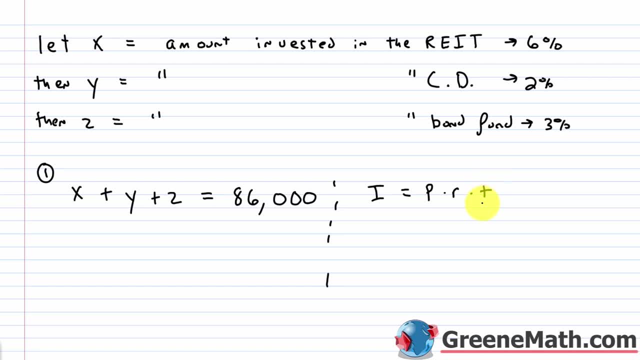 we're talking about annual, so that's one year. so if time is one, but multiplying by one, it doesn't change, so you just get rid of this. the thing about just principal times rate: now the principal or the amount invested in each case is listed with a variable. so if i take the reit, for example, 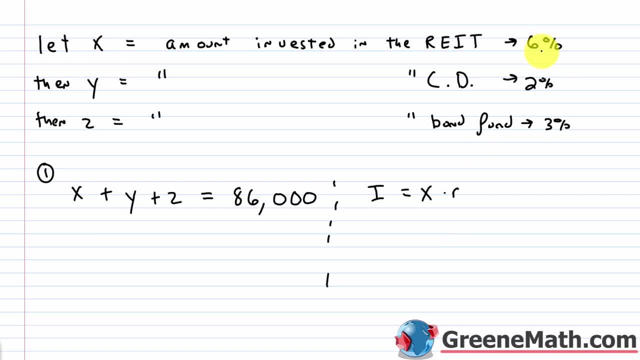 that would be x. now the rate i'm given is six percent. you got to write that as a decimal, so that would be 0.06. so let's rearrange this and put 0.06, so then times x. so i'm not given the. 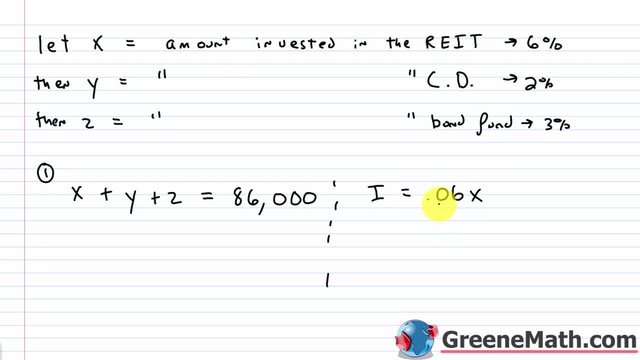 simple interest earned for just the reit. so this 0.06 x equals i. i don't know what i is for that, but that's fine. and then you know, i4 or the 3900 is this guy the reit plus the cd plus the bond fund. so my equation would be: 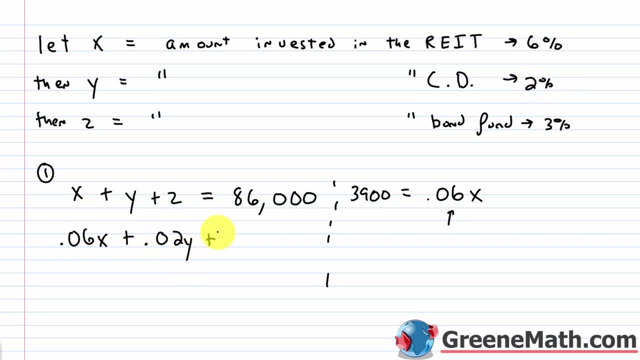 0.06x, plus the cd pays two percent, so point zero two y, plus the bond fund pays three percent, so point zero three z, and let me erase all this to $3,900.. And again, this comes from the simple interest formula. I have a 6% interest rate. 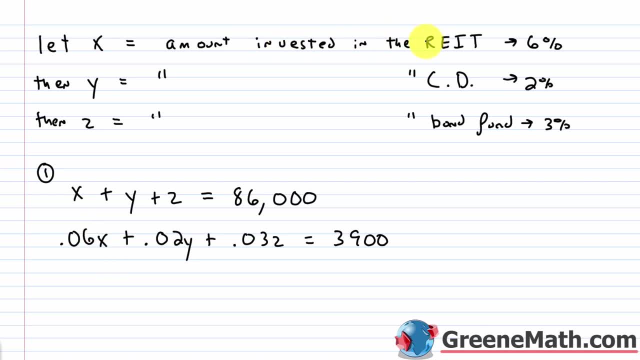 times an amount invested of X for my REIT. So if I multiply these two together, I'm going to get the amount of interest that's earned from the REIT in one year. I add that to the amount of interest that's earned from the CD for one year. I add that to the amount of interest that's earned. 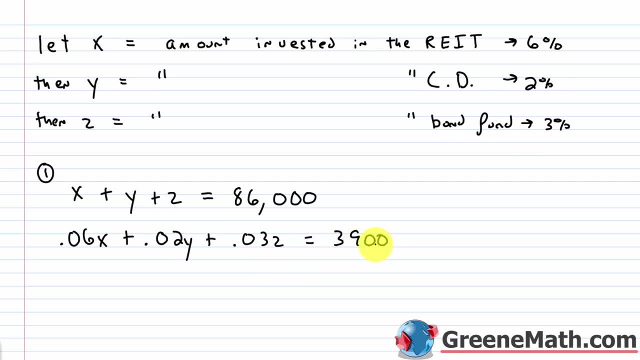 from the bond fund for a year And the total, as it's told to me in the problem, is $3,900.. So this is my equation two. Let's see if we can get a third equation. So we're told here that the 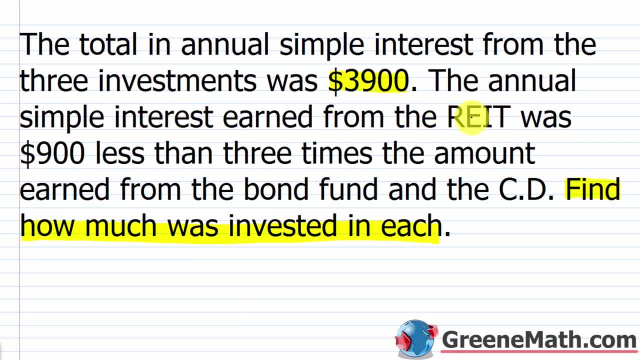 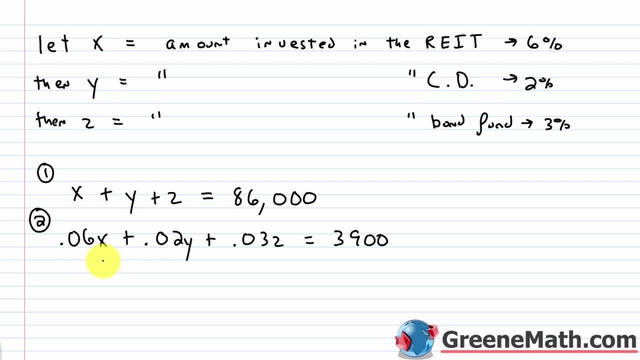 annual simple interest earned from the REIT. Let's stop. What was that? Well, we just saw that we put 0.06X for that right. 0.06 is 6% as a decimal. It's multiplied by X, which is the. 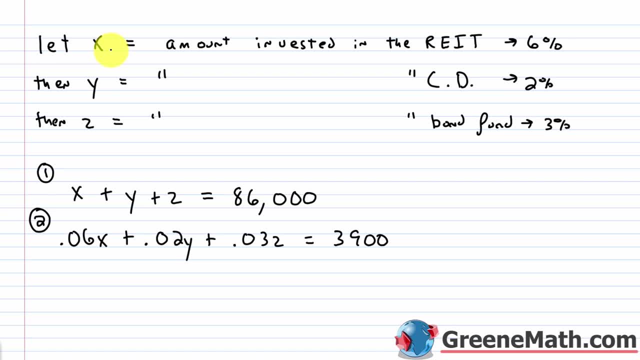 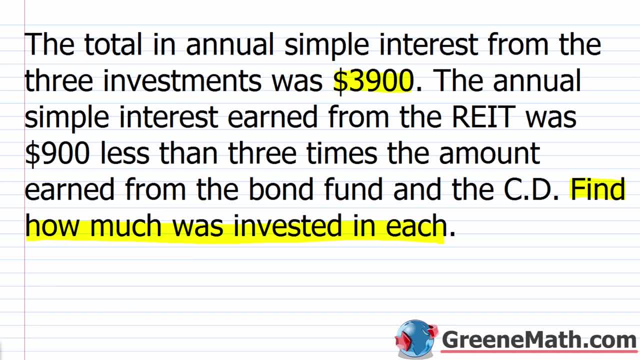 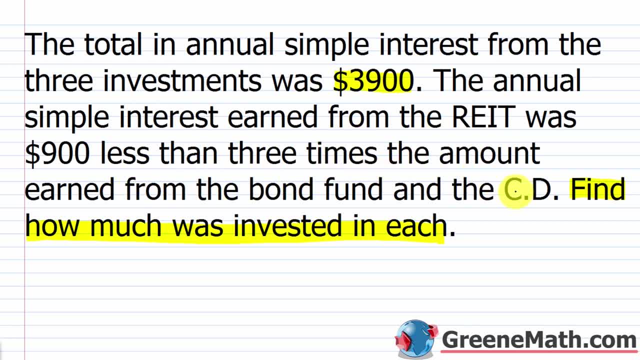 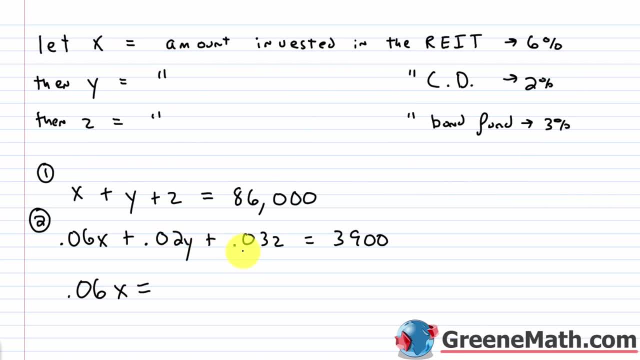 amount earned from the bond fund and the CD. So let's start with what's earned from the bond fund and the CD. Well, the CD and the bond fund we have with these two amounts, So we can put 0.02Y. 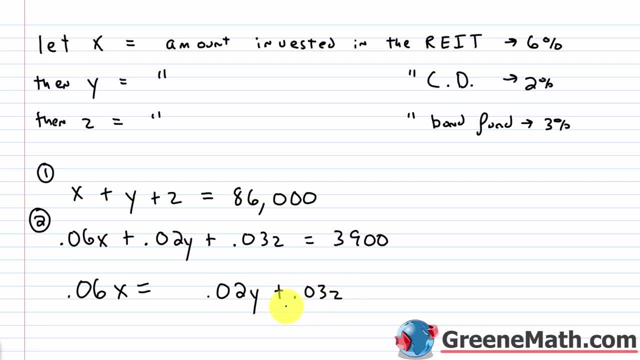 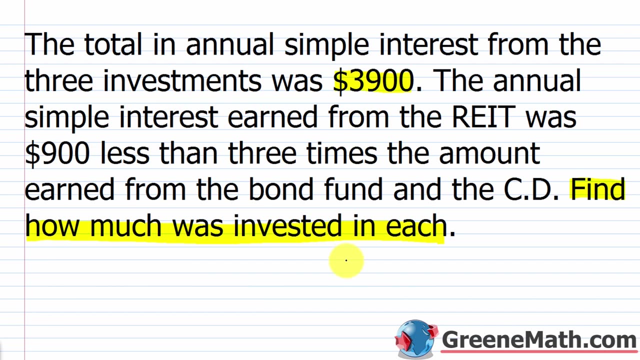 plus 0.03Z. Now it's three times this amount. So three times this quantity, and it's 900 less than that. So subtract away 900.. This would be my third equation. Let's go back up and make sure this makes sense. So again, and this is a little complex- 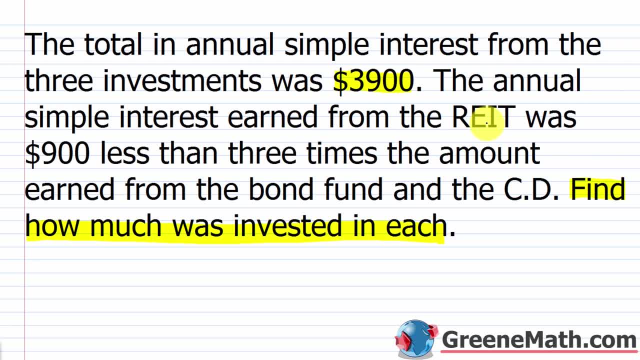 the annual simple interest earned from the REIT, which is 0.06X, was $900, less than three times the amount earned from the bond fund and the CD. So that's going to be 0.03X. So that's going to be. 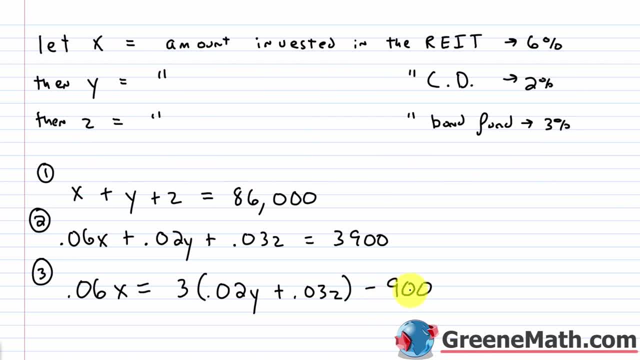 the amount earned from the bond fund and the CD. So we have 900. less than subtracting away 900 there, This is the amount earned from the bond fund and the CD. We have three times that amount. All right, So that's where that equation came from, And now we're ready to roll. Okay, So it. 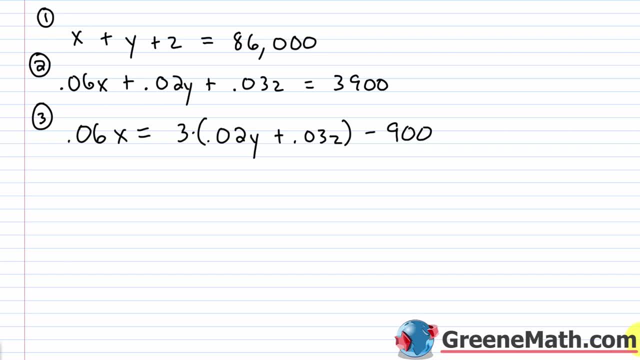 might take you a little while to get these three equations. when you first start You got to read through that problem very carefully. but I can assure you if this is in a textbook or on a test, the information is enough to get you the equations you need. They set it up that way. 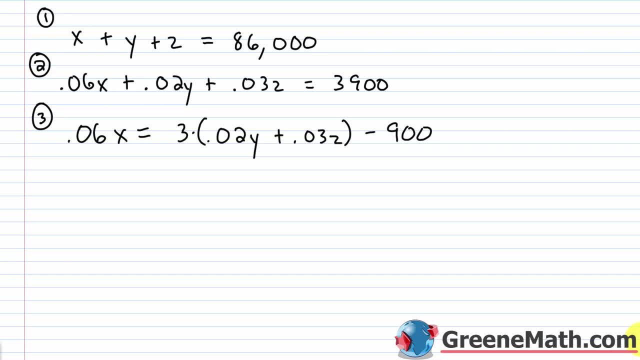 But sometimes it's not so straightforward what you need to do. So how do I want to solve this system? In most cases, with three equations, three variables, we eliminate a variable and then we solve a system in two variables And then we come back and we figure out the third. 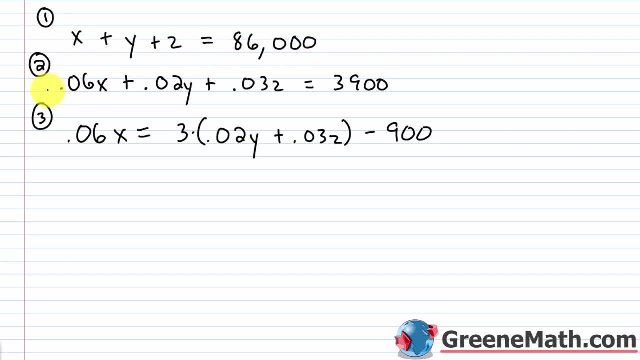 So let me just start with equation one and equation two. So equation one is: X plus Y plus Z equals 86,000.. Equation two: we have 0.06X plus 0.02Y plus 0.03Z: equals 3,900.. Now to make this easy. 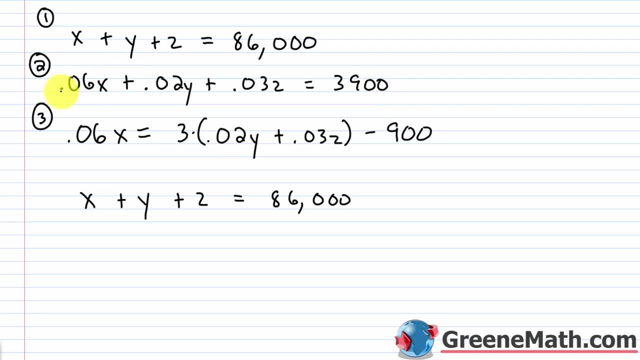 I can multiply both sides of this equation by 100.. Every decimal point would go over to the right by two, So this would be 6X plus 2Y plus 3Z equals, so in this case it'd be two zeros at. 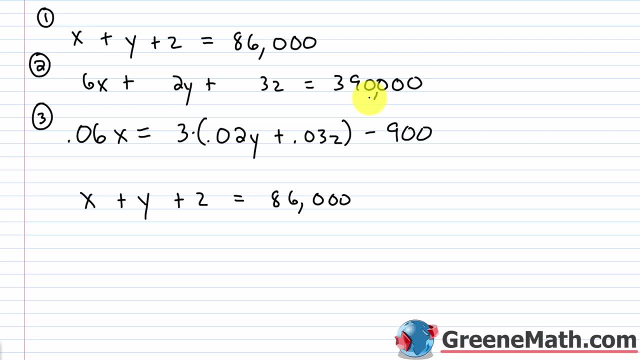 the end, So 390,000.. So we would have 6X plus 2Y plus 3Z- equals. so in this case it'd be two zeros at the end, So 390,000.. So we would have 6X plus 2Y plus 3Z- equals. so in this case it'd be two zeros at. 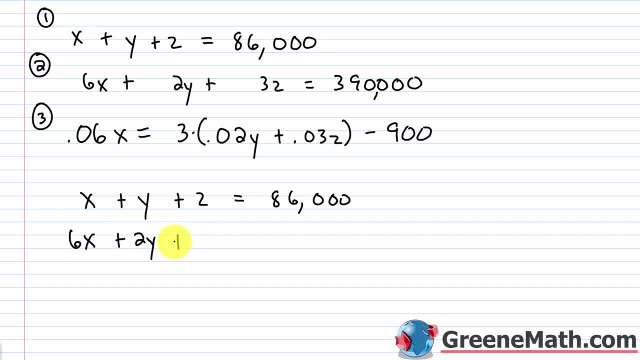 the end, So 390,000.. So we would have 6X plus 2Y plus 3Z- equals. so in this case it'd be two zeros at 6X plus 2Y plus 3Z equals. so in this case it'd be two zeros at the end, So 390,000.. Okay, So now. 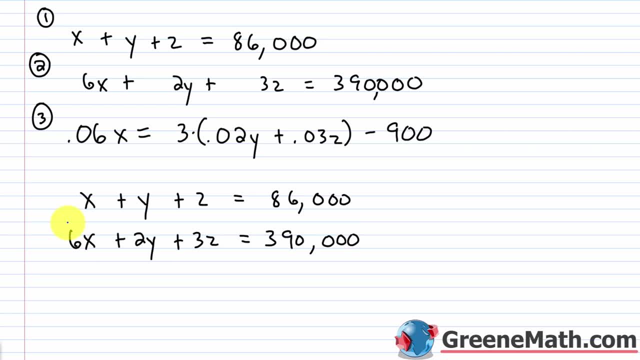 if I wanted to use elimination here, what I would do is just choose a variable. It doesn't matter what I choose, Let's go ahead and just choose Y. So if I want Y and 2Y to be opposites, what would 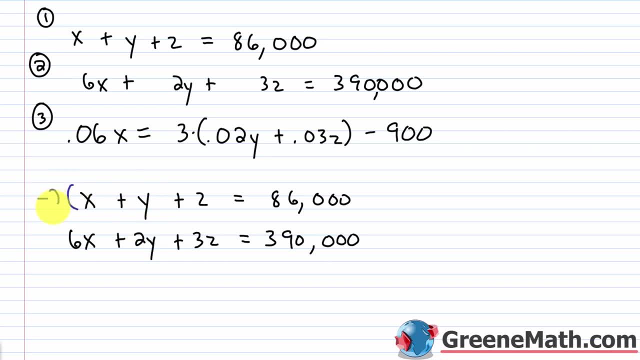 be easiest to make this negative 2Y. So let's multiply both sides of the equation by negative 2.. So negative 2 times X is negative 2X. Negative 2 times Y is minus 2Y. Negative 2 times Z is minus 2Z. This equals 86,000 times negative. 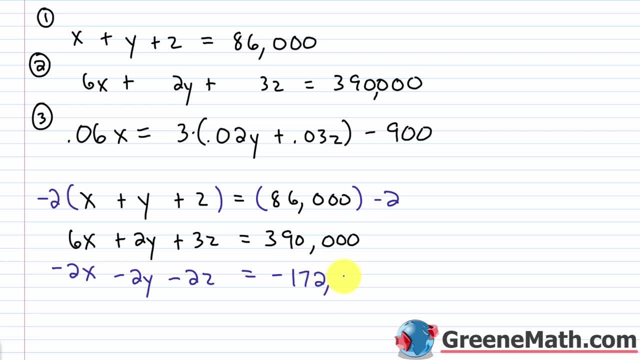 2. That's negative 172,000.. Let's erase this now. We don't need it anymore. So I can add the left sides together. Set this equal to the sum of the right sides. So 6X minus 2X is 4X 2Y minus 2Y. 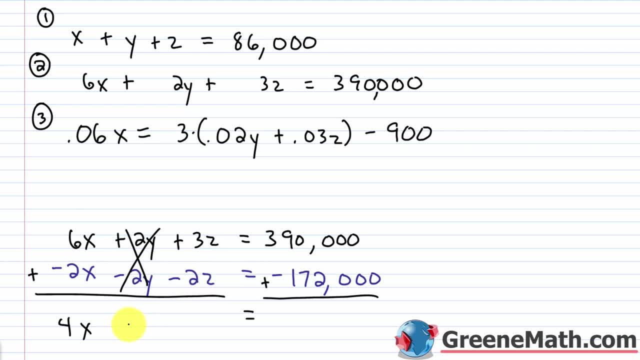 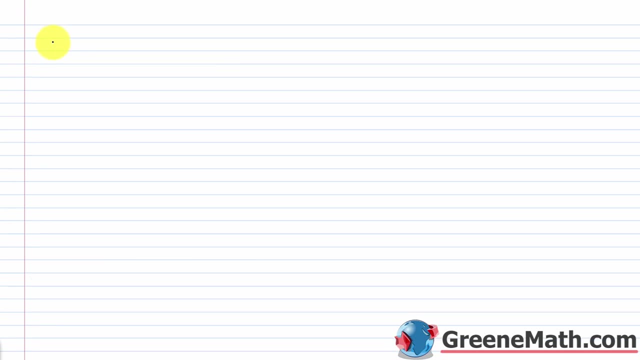 this is eliminated. 3Z minus 2Z is Z. So plus Z, 390,000 minus 172,000, that's going to give me 218,000. So this would be equation four. Let's write this on a new sheet. So equation four is: 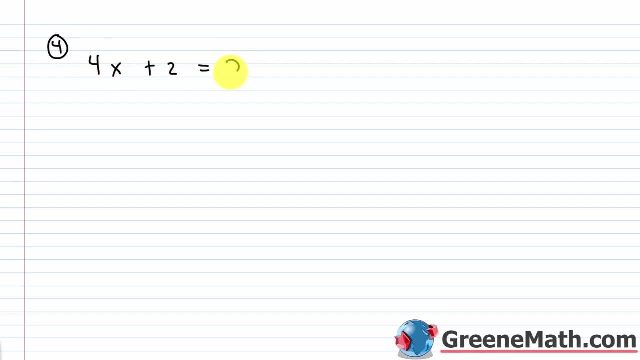 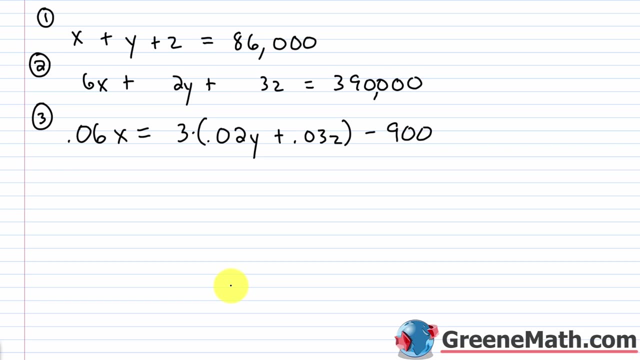 4X plus Z equals 218,000.. All right, let's go back up. All right, now let's work with equation two and three, And again we've got to eliminate the same variable this time. So we've got to eliminate. 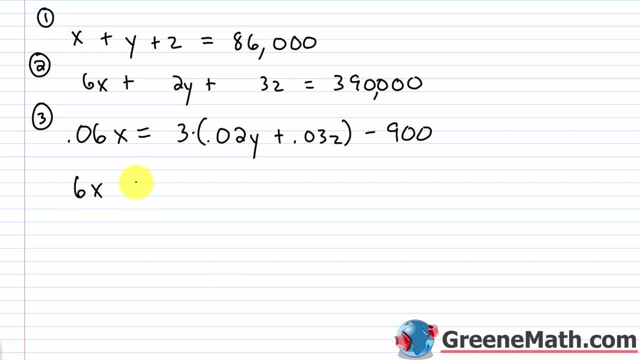 Y. So for equation two, I have 6X plus 2Y plus 3Z equals 390,000.. For equation three: it's a little clustered, Let's kind of clean it up. So 0.06X equals 3 times 0.02 is 0.06,. 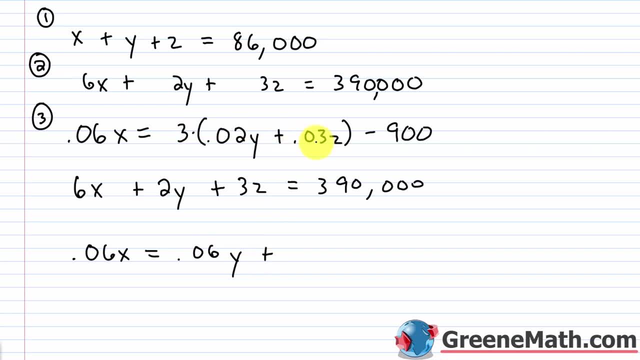 then times Y plus 3 times 0.03 is 0.06.. 0.09, then times Z, then minus 900.. Now again I can clear the decimals by multiplying everything by 100. So this would go two places to the right. That would be 6X. This goes two places to the. 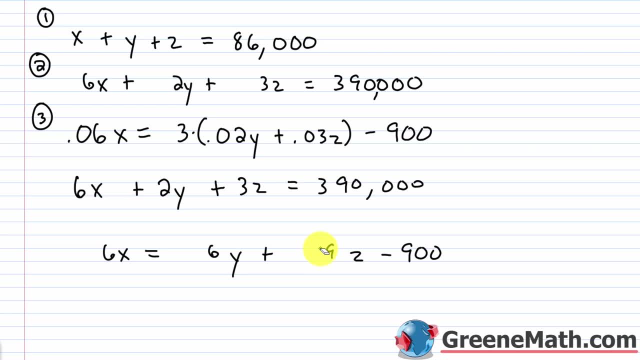 right, It'd be 6Y, This would be 9Z, And I'd put two zeros at the end here to give me 90,000.. So I can erase this And let me just write it in this format. So I'd have 6X. 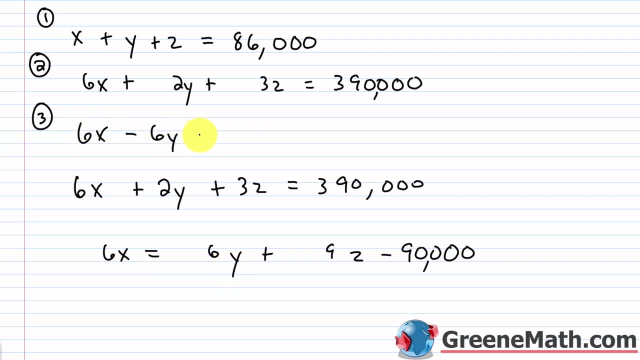 Let me subtract. Let me subtract away 6Y from each side, Let me subtract away 9Z from each side, And this will equal negative 90,000.. Okay, So let me erase this, And so I'll write 6X. 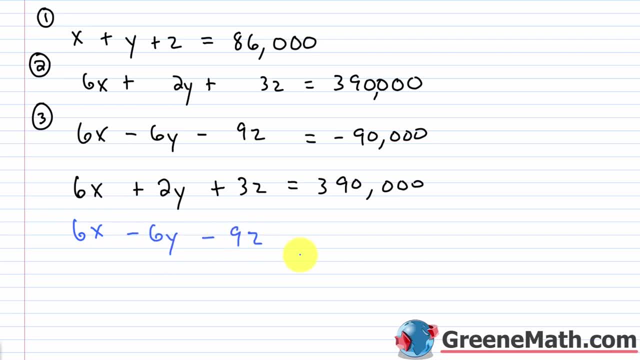 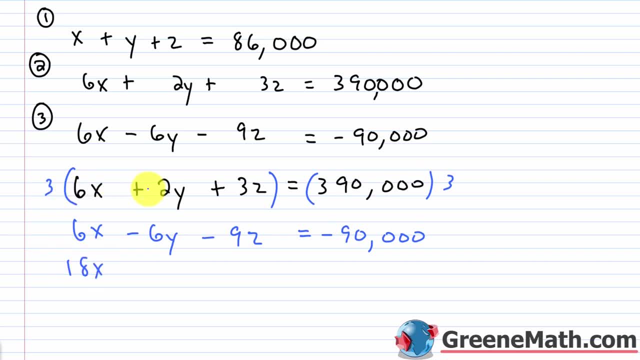 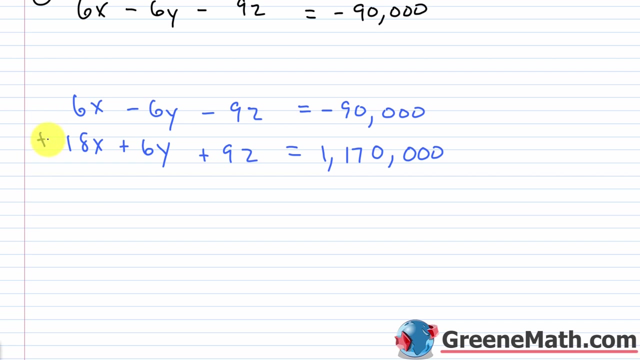 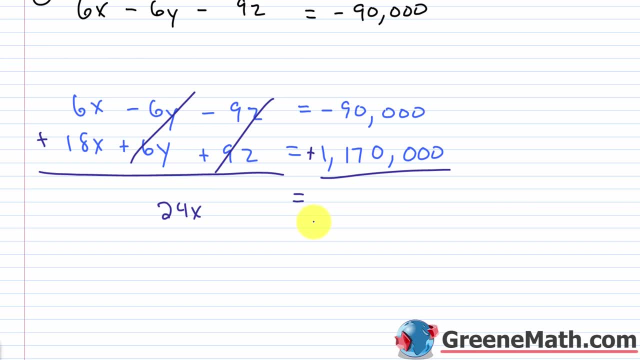 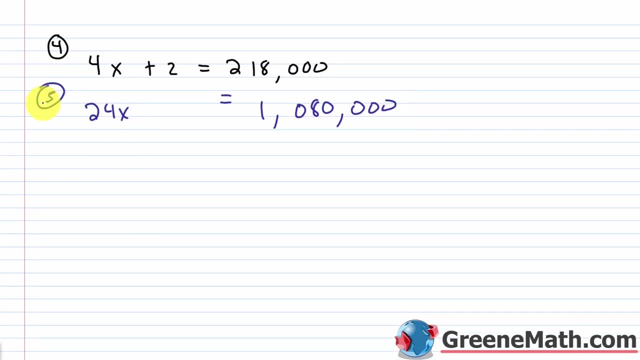 6x plus 18x is 24x, And this equals negative. 90,000 plus 1,170,000 is 1,080,000.. All right, so let's copy this. That'll be equation five. Let me kind of tighten this down a little bit, So it's pretty easy. We're just going to solve this equation five for x, So we would get x as. 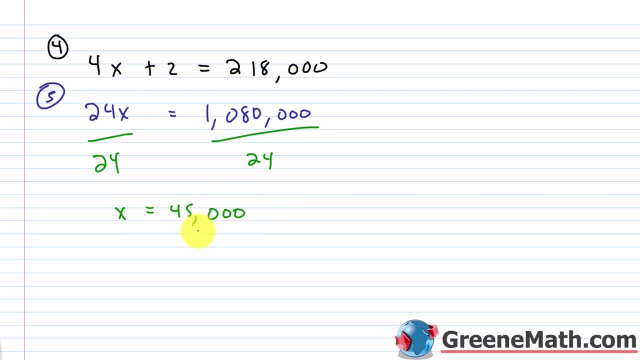 equal to 45,000.. Now I'm going to plug 45,000 in for x in equation four, So I would have: four times 45,000 plus z is equal to 218,000.. Four times 45,000 is 180,000, plus z equals 218,000. 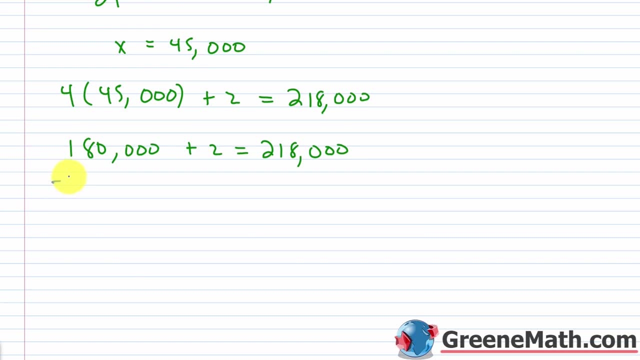 Scroll down. get a little room going, Let's go ahead and subtract 180,000 from each side of the equation. That'll cancel. We'll have z is equal to 38,000.. All right, So now I know x is. 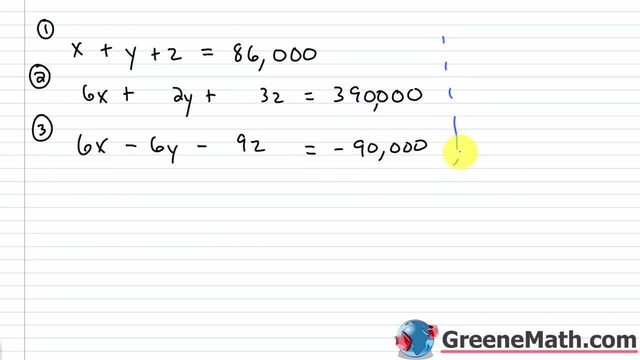 45,000.. I know z is 38,000.. So we know z is 38,000.. X is 45,000.. Let's just plug that into equation one. So we'd have 45,000 plus. 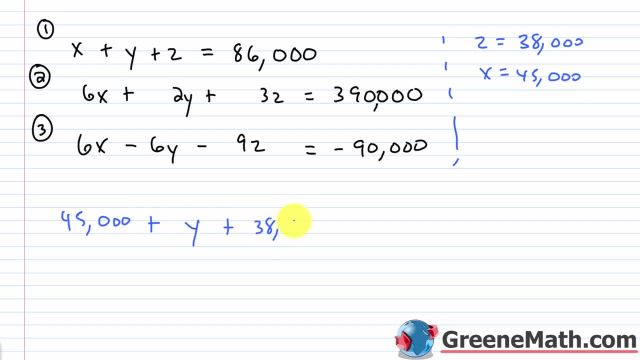 y plus for z 38,000. This equals 86,000.. So if I had 45,000 and 38,000, I'd get 83,000.. So you'd have y plus, 83,000 equals 86,000.. Go ahead and subtract 83,000 away from each side of the. 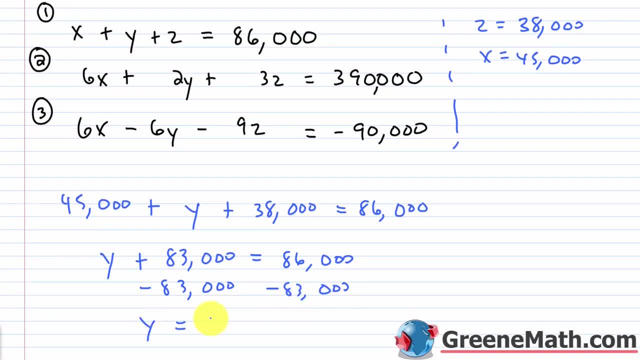 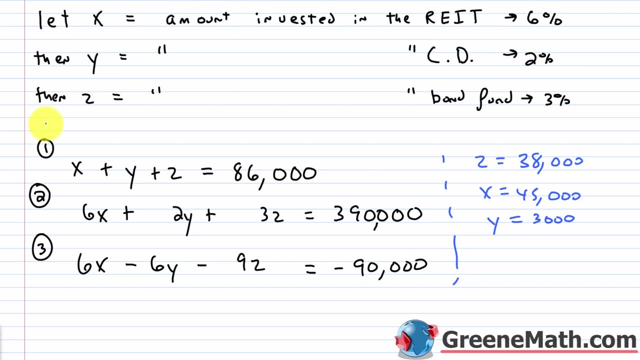 equation: Y is going to equal 3,000.. So y equals 3,000.. Okay, So now I want you to remember what x, y and z represent. X is the amount invested in the REIT. Y is the amount invested in the CD. Z is the amount invested in the bond fund. 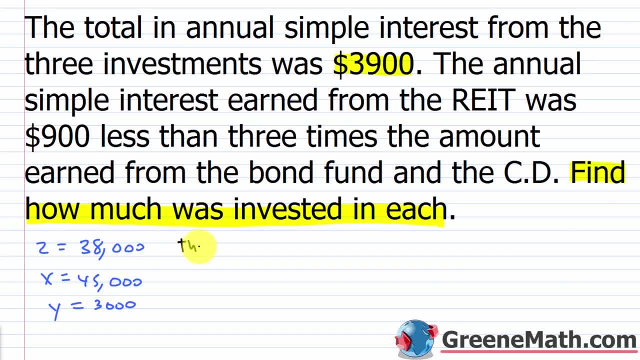 So let's take this up. We're going to say there was $45,000 invested in the REIT and $38,000 invested in the CD and $38,000 invested in the bond fund. Now again, if you check this, 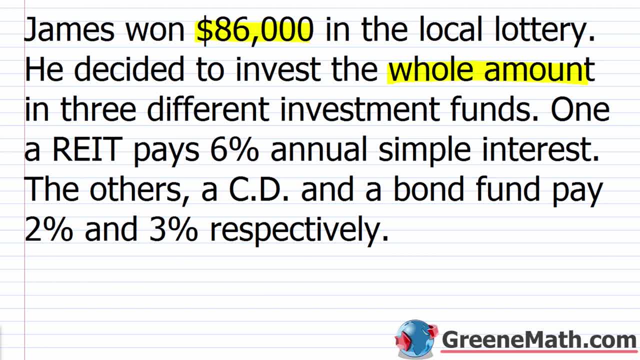 you think about, James invested $86,000.. This is the amount he invested, So let's take that out to total. So is that consistent with what you found? Well, $45,000 plus $38,000 is $83,000 plus another. 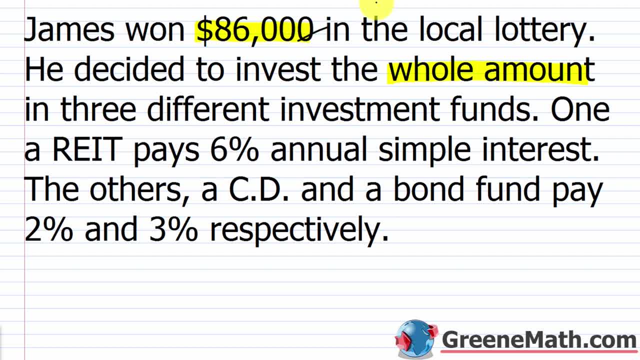 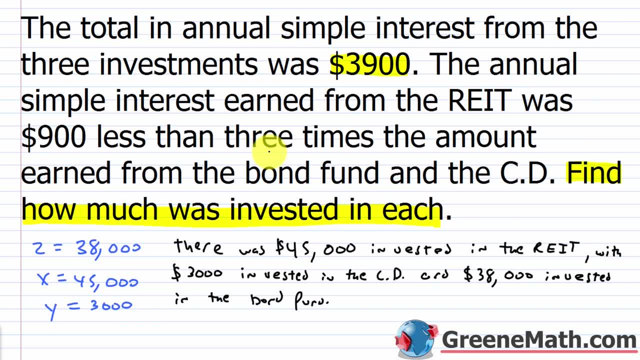 $3,000 is $86,000. So it checks out there. Now the next thing is the total annual simple interest from the three investments is $3,900.. Does that work out Well from the REIT you've? 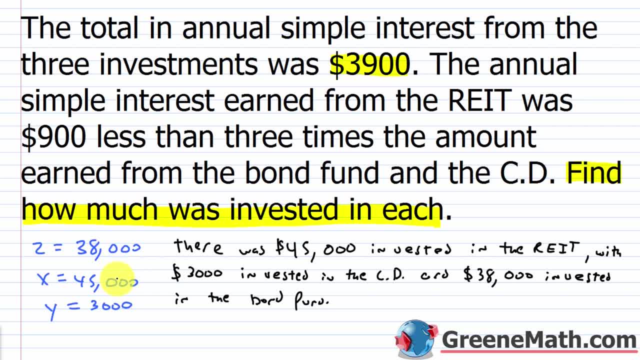 got $45,000 invested at 6%, That's $2,700. in interest In the CD, it's $3,000 at 2%, so that's $60.. And then if you take the bond fund, that's $38,000 at 3%, That's $1,140.. So if you add, 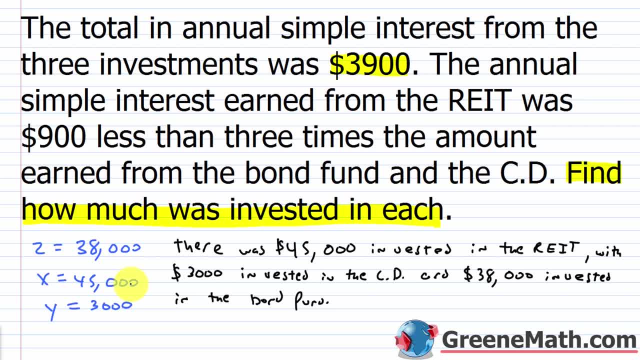 $2,700 plus $60, you would get $2,760 plus $1,140.. You do in fact get $3,900.. So it checks out here as well. now the last one. it says the annual simple interest earned from the reit, which. 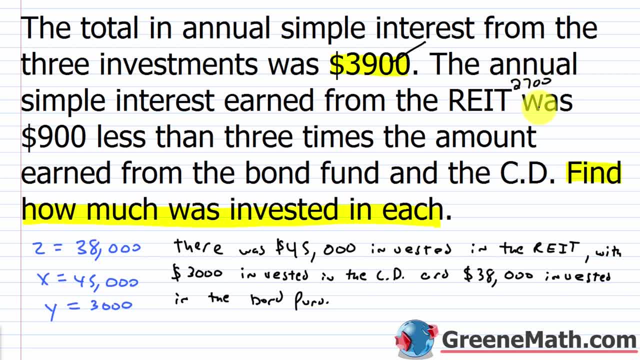 is twenty seven hundred dollars, was nine hundred dollars, less than three times the amount earned from the bond fund and the cd. so from the bond fund he got eleven hundred forty dollars, from the cd he got 60. so combine those two amounts together you get twelve hundred. so again it was. 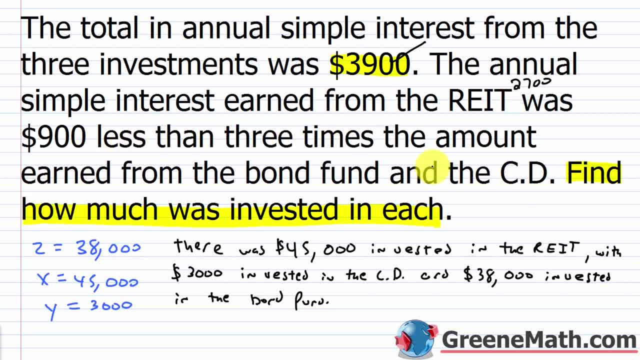 nine hundred dollars, less than three times the amount of twelve hundred dollars. three times twelve hundred would be thirty six hundred. thirty six hundred minus nine hundred would be twenty seven hundred, so that one checks out as well. so a very tedious problem overall. takes a little bit time to get into it, takes some time to set up and take some time to check it, but worth it in the end. 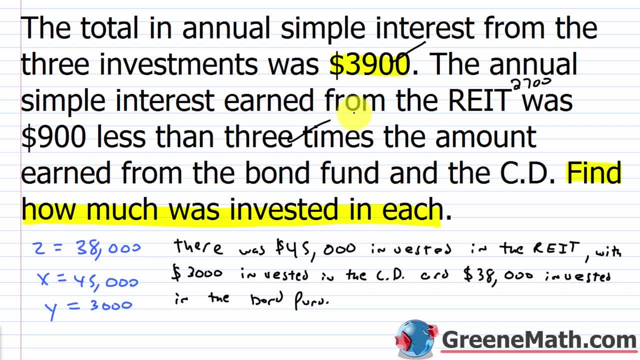 because you've got to see a few of these, because if you get them on a test you can't just be, you know, completely rattled. okay, you had some experience now in dealing with one of these really tedious problems. so again, to just state the answer: there was forty five thousand dollars invested in the reit, with three thousand. 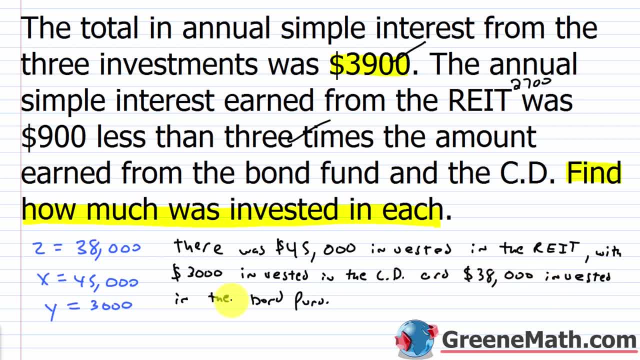 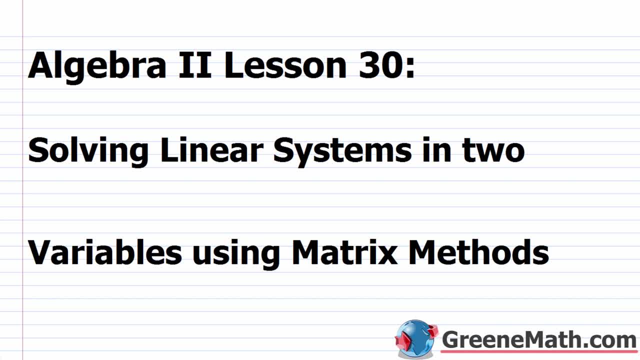 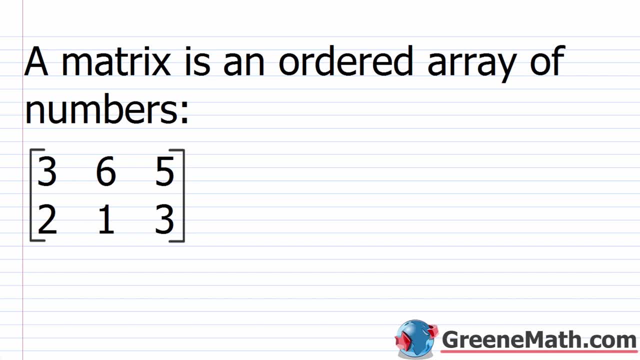 dollars invested in the cd and thirty eight thousand dollars invested in the bond fund. hello and welcome to algebra 2, lesson 30. in this video we're going to learn about solving linear systems in two variables using matrix methods. so in this lesson i want to talk a little bit. 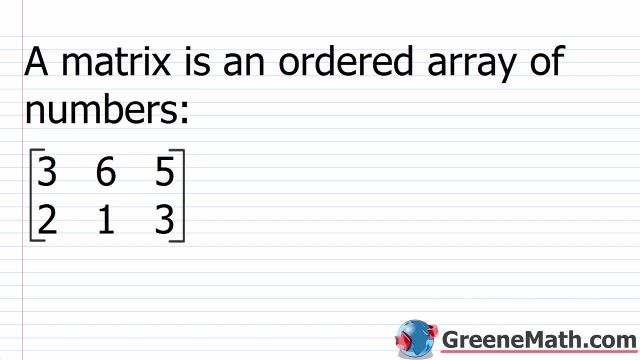 about another method used to solve linear systems in two variables using matrix methods. so so far we've learned how to use graphing, substitution and elimination. but we're going to push ourselves a little bit further and now talk about matrix methods. so as we move higher in math, 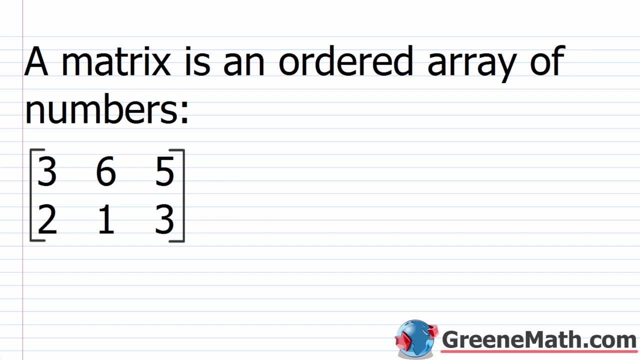 things are going to become more complex. matrix methods allow for us to solve very large linear systems using a computer very, very quickly. so we're not going to cover all of the details related to a matrix, but what we will do is give an introduction and show one method for finding a solution using 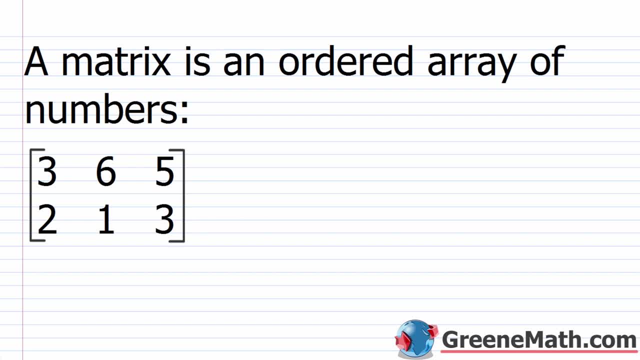 a matrix. so let's start out with the very basics here. so a matrix is an ordered array of numbers and it's just a way to store numerical information. so you'll see my brackets here and in the brackets you have two rows. okay, two rows. this would be a row going across. We have two rows- okay, two rows- of Gone I Eighths to the Eighths. so we have a square on a and then a square on the In thurs and a F Achievement type. So if time be Format less than zero, then we don't have enough to have. So we don't need a killing and if times are right, the same later on. 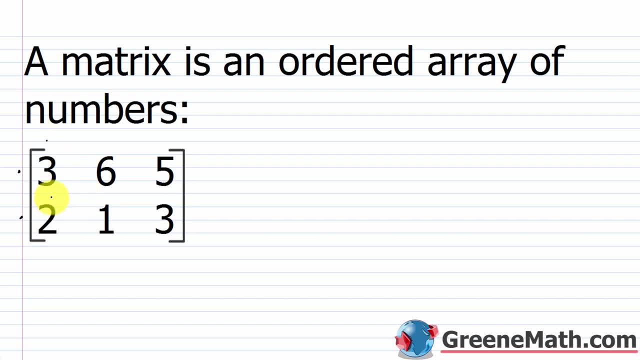 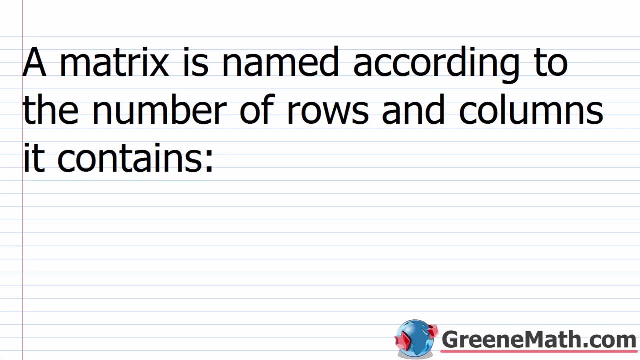 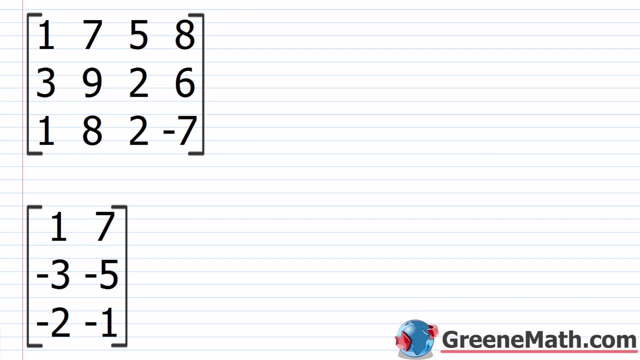 two of those and you have three columns, So the columns are going down. So a matrix is named according to the number of rows and columns it contains. It's rows first, followed by columns. So, as an example, if I see this matrix here, you see that you have one, two, three rows, So three. 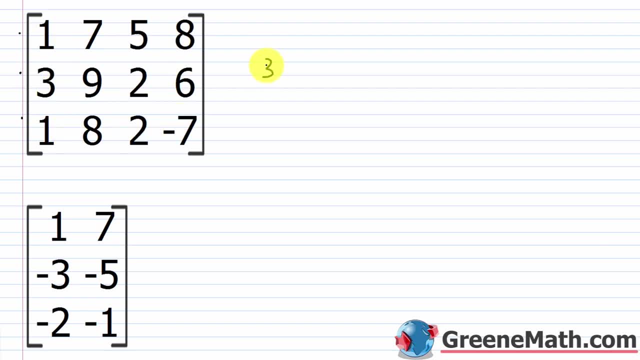 going across. So three is the first number and you have one, two, three, four columns, So four is the second number. So this is a three by four matrix. Similarly, with this guy right here, you have one, two, three rows, So it's a three rows there, and you have one, two columns, So this is a three by two. 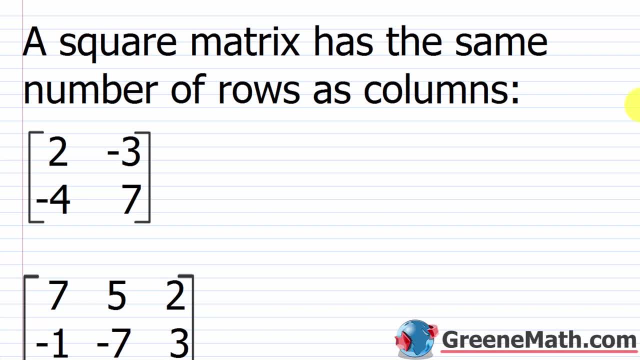 matrix. So another little kind of definition that you'll come across. you have a square matrix. Let me highlight that A square matrix has the same number of rows as columns. So here I have two rows and two columns. So this is a two by two matrix. As another example of a square matrix, 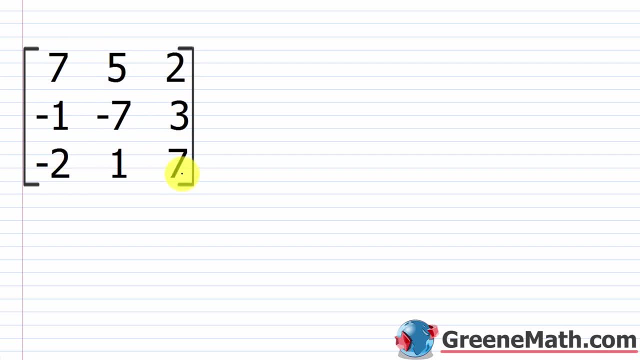 we have three rows here and we have three columns, So this is a three by three right. You can have anything by anything, So you can have four by four or 27 by 27, as complex as you want to make that. 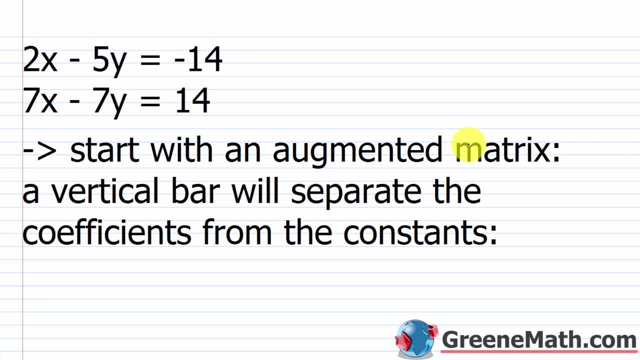 All right. so I want to start out today with a very basic example. So we have the linear system: 2x minus 5y equals negative 14.. We have 7x minus 7y equals 14.. I have here start with an augmented 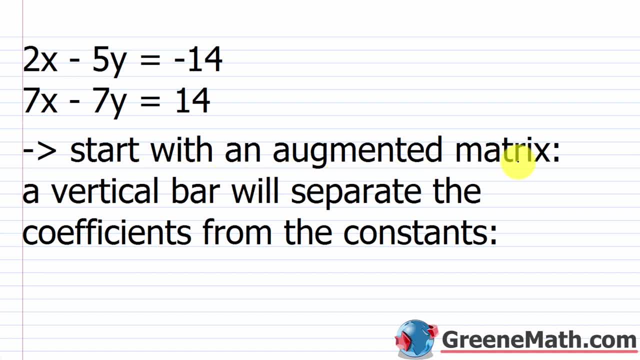 matrix. Before we get into that, I want you to notice that we have each equation already written in standard form. So you want to start by putting ax plus by is equal to c, Both equations in the standard form. Now, once you've done that, you can write this augmented matrix, What this is. 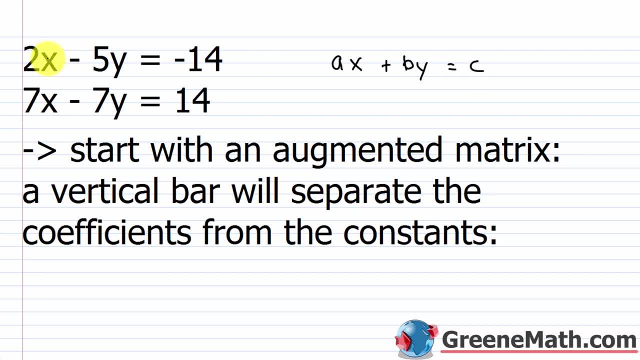 is. I'm going to take the numerical information only. So, in other words, the coefficient for x is a 2. So I'm going to write a 2.. The coefficient for y here is a negative 5.. So I'm going to write. 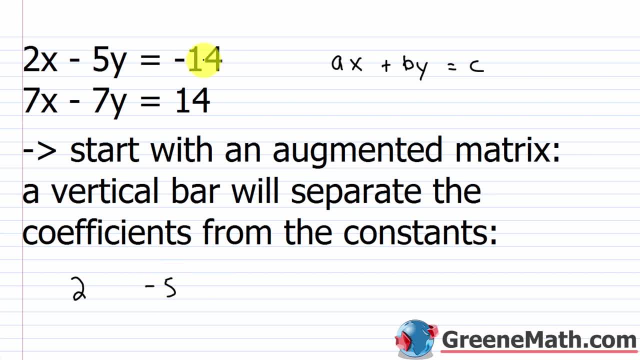 negative 5.. The constant is negative 14.. So I'm going to write negative 14 there. So that's my first row. It represents the numerical information from the first equation of the system. My second row is the same thing. So I have a 7 for x, I have a negative 7 for y And I have a 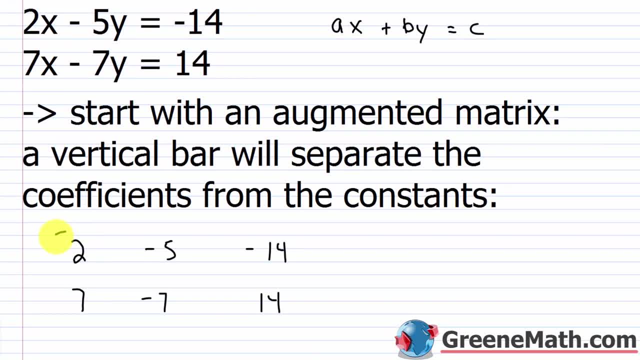 positive 14 as my constant. Now I'm going to put my brackets here And with the augmented matrix we use a vertical bar to separate the coefficients from the constants. So my coefficients are here, These are the coefficients And these are my constants. So I'm just going to put a vertical bar. 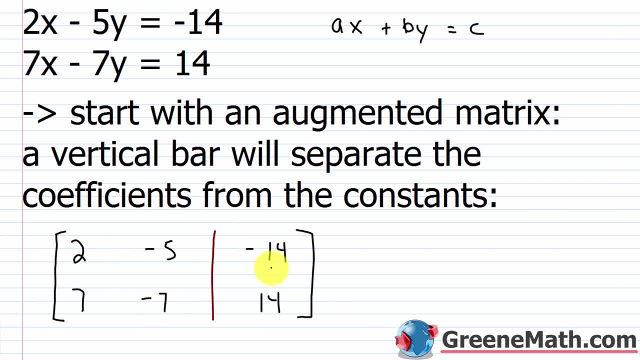 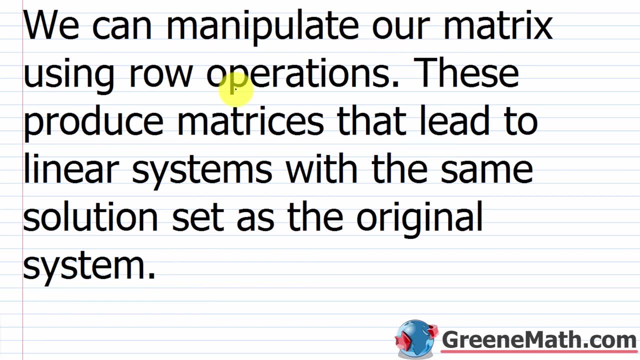 right here. So from this information here, we can get a solution for x and y. Now, in order to do that, we're going to use these elementary row operations, And there's three of them, So let's go ahead and look at that. All right, So I have here. we can manipulate our matrix using row operations. 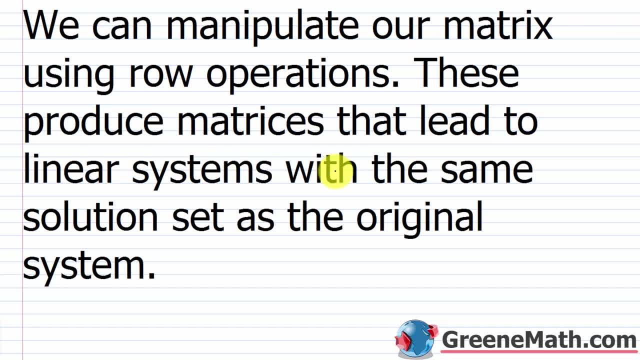 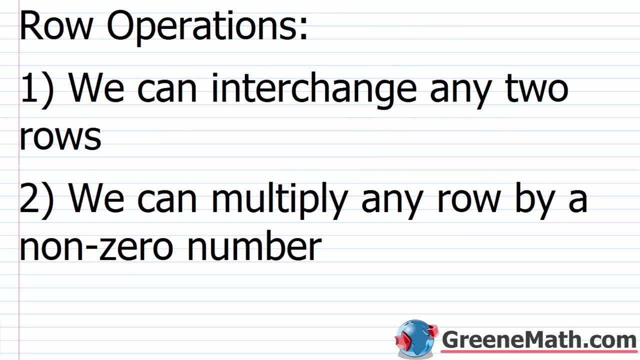 These produce matrices that lead to linear systems with the same solution set as the original system. All right, So here's our row operations. The first thing is that we can interchange any rows. That makes sense, because if I had an equation and another equation, it doesn't matter. 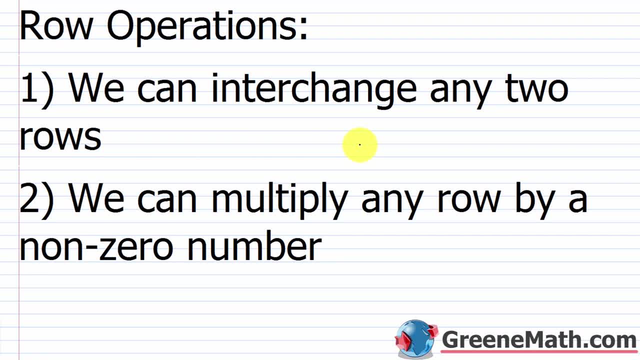 which one I write on top. I can switch that around as much as I want. The second thing is: we can multiply any row by a non-zero number. Well, that makes sense. I can multiply both sides of an equation by a non-zero number. I could divide both sides of an equation by a non-zero number. 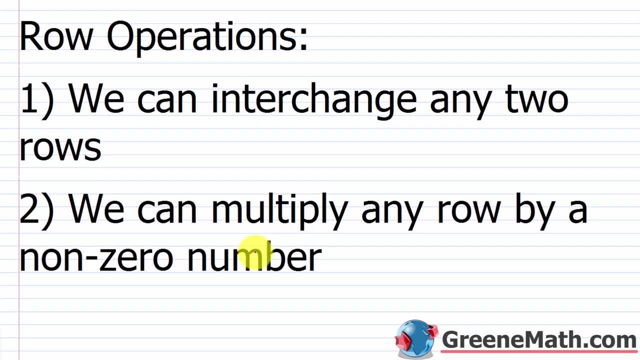 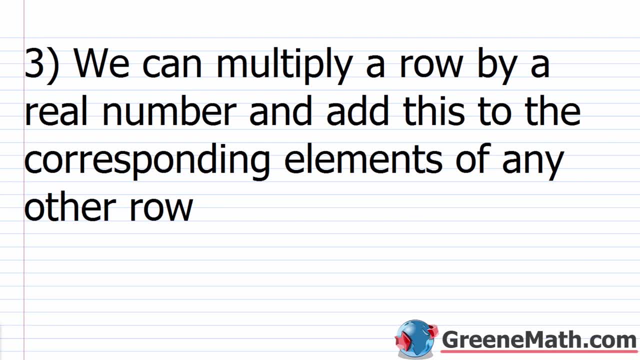 And the equation would contain the same solution set. So the last row operation- we're going to talk about row operation 3, is a little bit challenging to understand. So we're going to talk about row operation 3.. So we have here that we can multiply a row by a real number and add 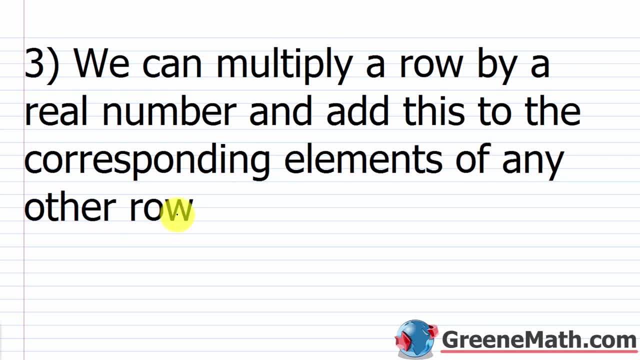 this to the corresponding elements of any other row. So when people first see this, they say: well, what makes this legal? Well, essentially we're using the same basic principles that we use when we use the elimination method. So we're going to quickly look at a different example. 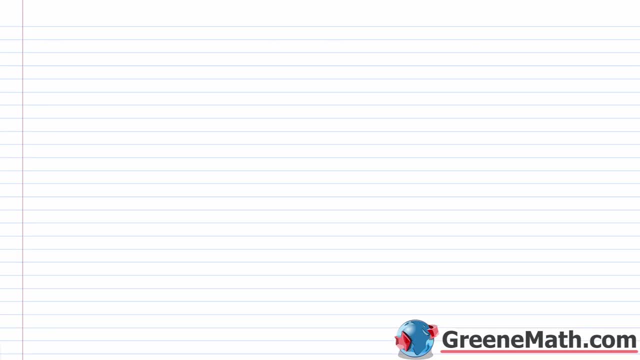 And I want to just cover why this would work. So let me just take an aside from that problem that we're currently working on. So just put that to the side, take out a fresh sheet of paper and I want you to work through this very basic example with me. 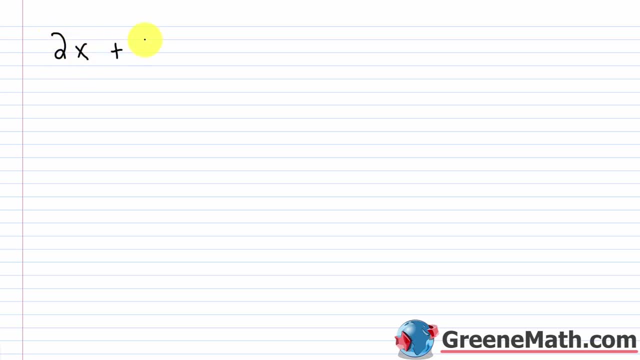 So if we have 2x plus 3y equals 11, and we have x plus 2y equals 7.. So we can easily solve this using elimination at this point. So I want to do elimination and I want to do the matrix. 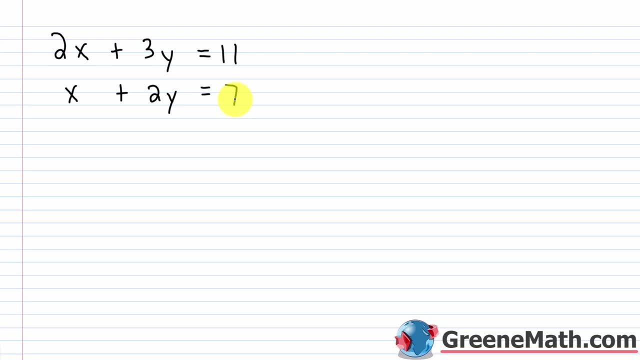 method. I'm not going to go all the way through it, I'm just going to go to the part where it's obvious what the solution is. So if I wanted to solve this with elimination, what would I do? Let's go ahead and say this is equation 1, and this is equation 2.. Well, I know that I can. 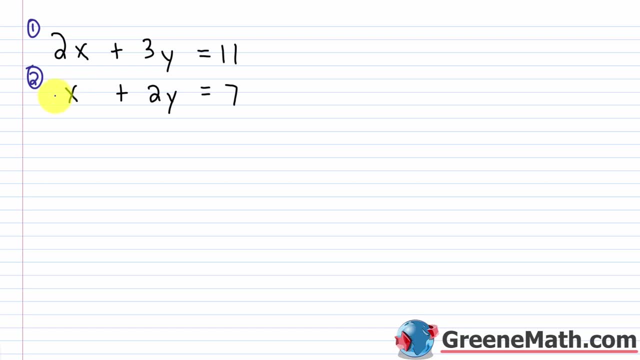 eliminate x if this was negative 2 here. And the way I can do that is I can multiply both sides of this equation by negative 2.. So if I did that, what I would have is a negative 2x plus negative 4y equals negative 14.. So I could write that I have 2x plus 3y equals 11,. 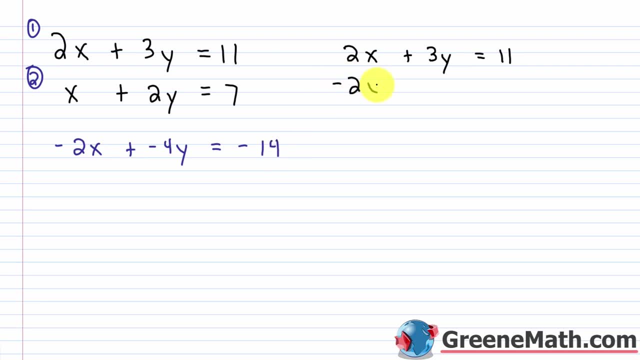 and I have this other one: negative 2x minus 4y is equal to negative 14.. Okay, So now we all know at this point that the x variable would be eliminated, So I could add the two left sides of the equation. 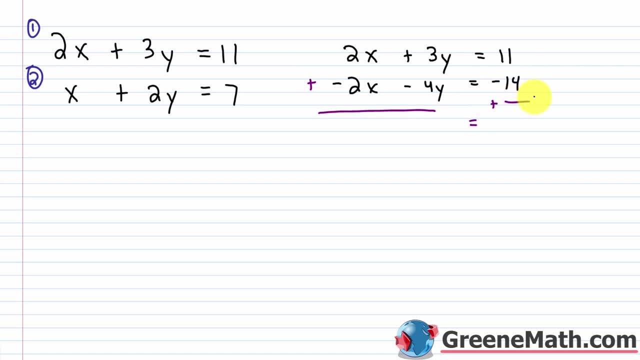 Set that equal to the sum of the right sides of the equation. So 2x minus 2x would be 0.. x is eliminated. That's gone. 3y minus 4y is negative y And this is equal to. let me kind, 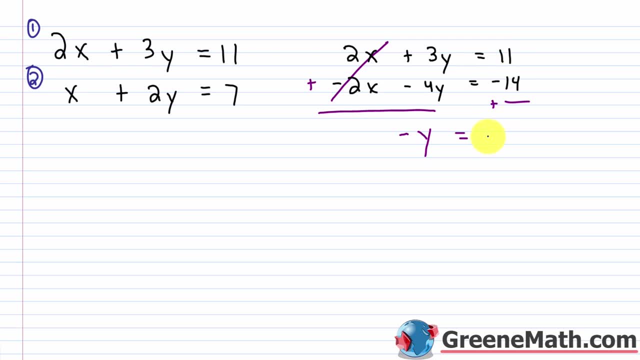 of move this down a little bit: 11 minus 14, which would be negative 3.. So we all know that y is 3.. So y is 3.. Now I can plug a 3 back in here and figure out what x is. 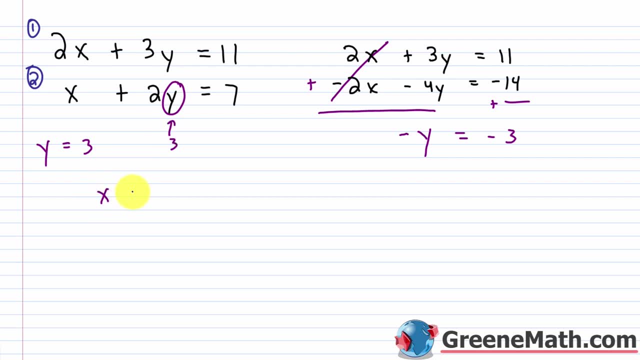 2 times 3 is 6.. So I would have x plus 6 equals 7.. We know x would be 1, right, x is equal to 1.. Now I want to just show you this real quick using a matrix, so I can relate the steps. 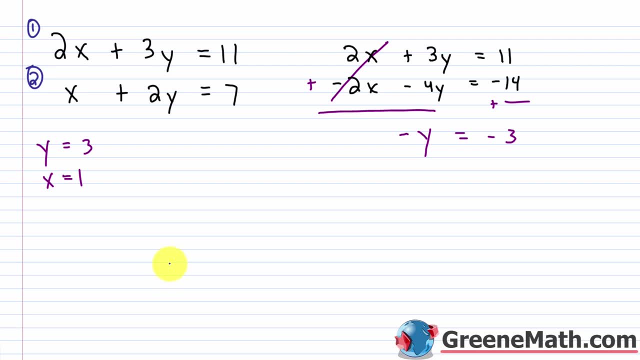 So the first thing is we want an augmented matrix. So I just told you. we take the numerical information Again. these equations are written in standard form: ax plus by equals c. So So I have my coefficient for x, my coefficient for y and my constant, written in that order. 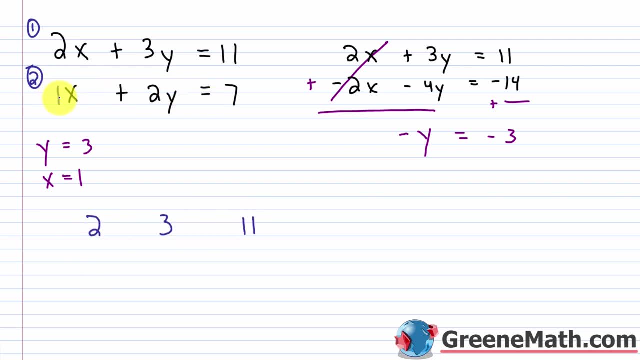 I'm going to write it in the same order here, So this is understood to be a 1, so just a 1,, a 2, and a 7.. I've got a vertical bar that separates the coefficients from the constants. 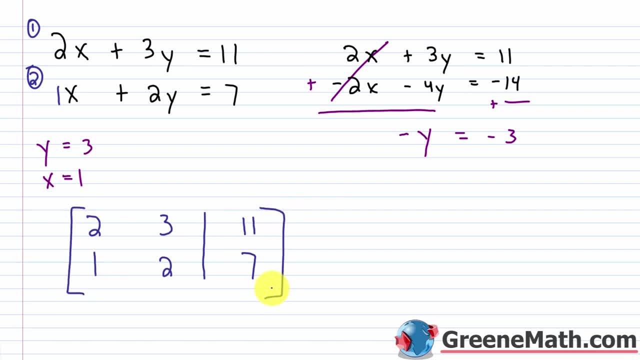 Now, using the numerical information only, I can do the same thing that I did here. I want to think about how could I get a 0 here, so that the coefficient for x is a 0, and x is essentially eliminated. I would have some number times y equals some value, which is what I had here. 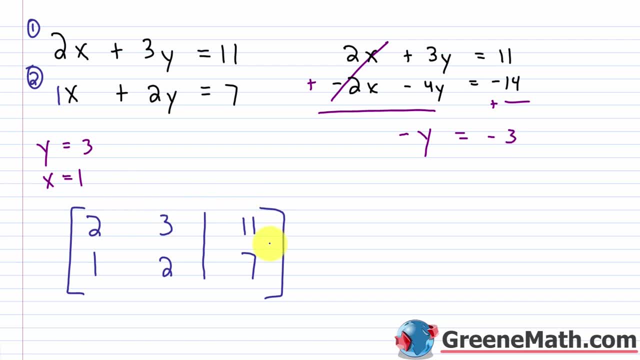 So I'm going to show you that I can use the elementary row operations. I can say: if I multiplied row 2 here by negative 2, which is exactly what I did here- Remember Second equation- I multiplied it by negative 2, and I produced negative 2x minus 4y equals. 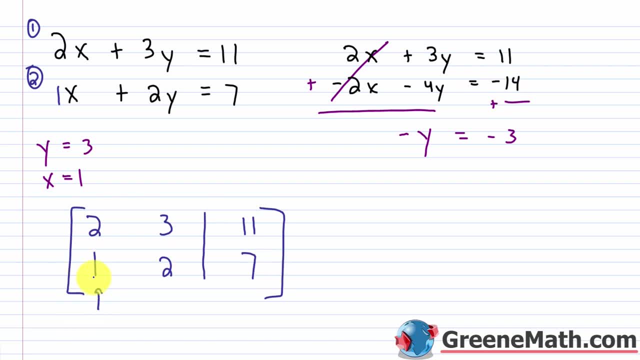 negative 14.. So if I multiplied row 2 by negative 2, 1 times negative, 2 is negative 2, 2 times negative 2 is negative. 4, 7 times negative 2 is negative 14. And then I added those elements to row 1.. 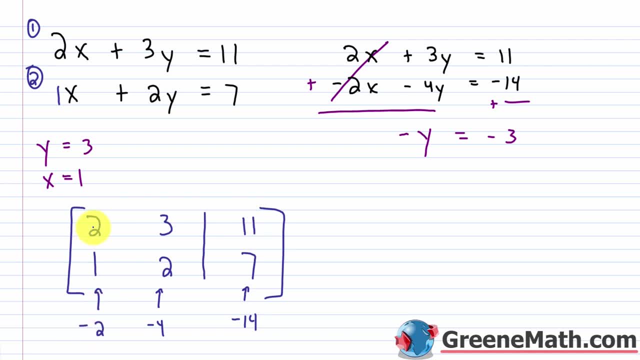 So negative 2 plus 2 would be 1. That would be 0. So I'd have a 0 here. Then negative 4 plus 3 would be negative 1, then negative 14 plus 11 would be negative 3.. 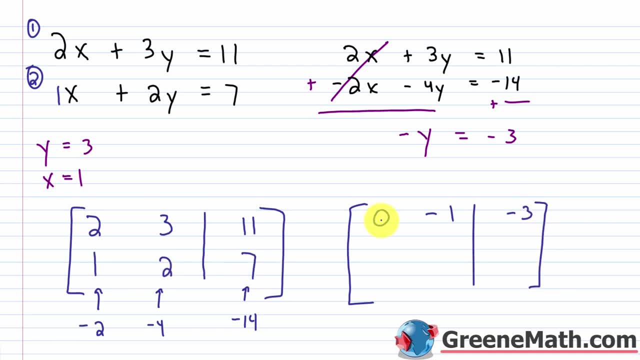 Now, I don't need to change this row here because I already have what I need there, So I can just leave this as 1, 2, and 7,. okay, But it wouldn't matter if I wrote negative 2,, negative 4, and negative 14 there. 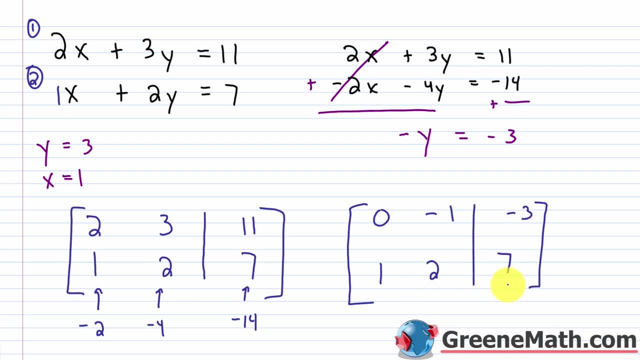 But for the purposes of working with a matrix, we're not going to do that. We're just going to leave this row unchanged. Now I have the same information here that I have here. I know that the coefficient of x is 0, so x is eliminated. 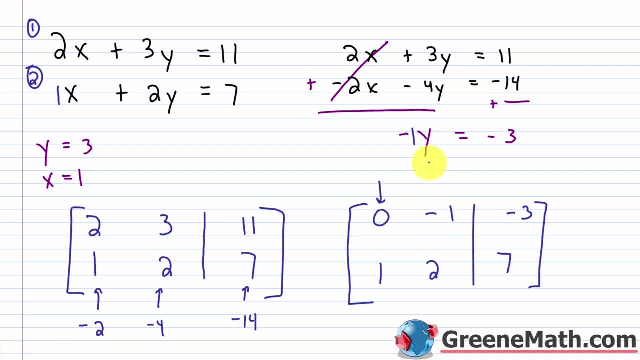 I know that the coefficient for y is negative 1, so basically I have negative 1y is equal to negative 3.. So from this information here I can solve for y okay, and then I can go back and figure out what x is. 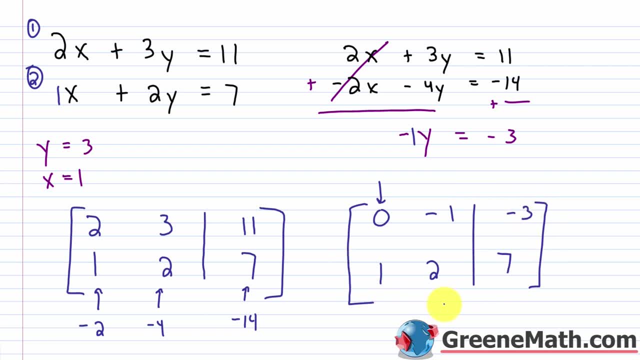 Now, This isn't exactly how we're going to solve u. This isn't exactly how we're going to solve u. This isn't exactly how we're going to solve hat. This isn't exactly how we're going to solve t. This isn't exactly how we're going to solve the quadratic formula. 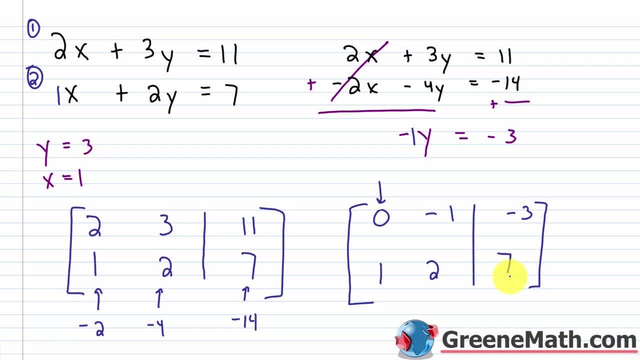 This isn't exactly how we're going to solve the quadratic formula, but we could use this formula as an example of how we can manipulate the numerical information to get a solution. So I want to return now to the official procedure. Again, this is just a little side note. 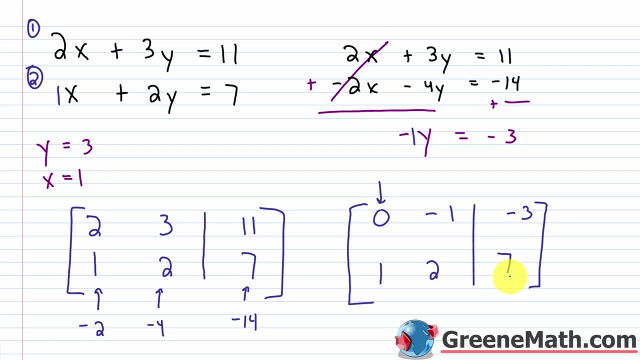 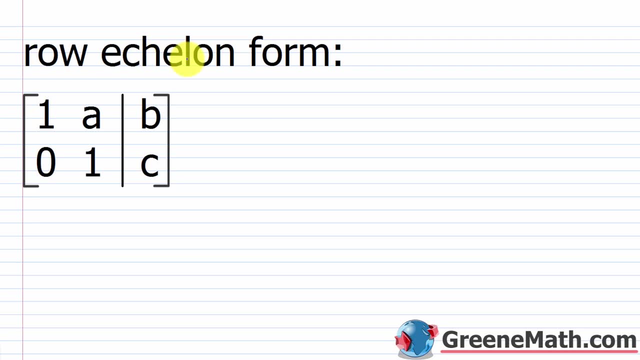 You can kind of get rid of this now And let's go back to the original problem: What our goal is actually going to be. We have this term known as row echelon form, And you're also going to hear reduced row echelon form. 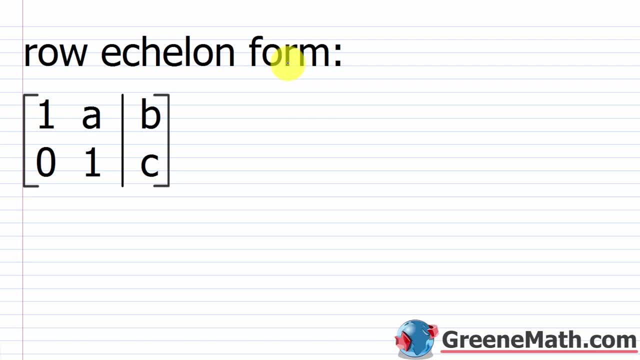 I'm going to cover both. I'm going to cover both of them, but I want to focus on row echelon form for now. So what you want is ones down the diagonal. So, starting at the top left, you have a one. then, going this way, you'd have another one. 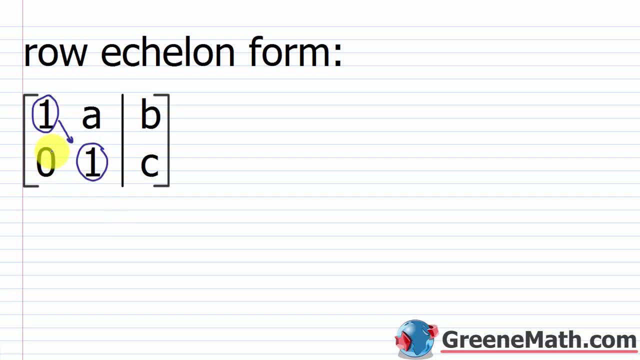 Now, beneath the ones you're going to put a zero. so this has to be a zero. Now you're going to have real numbers above and to the side. So this is a, b and c just representing real numbers. If I have something in row echelon form, and again these equations are ax plus by equals. 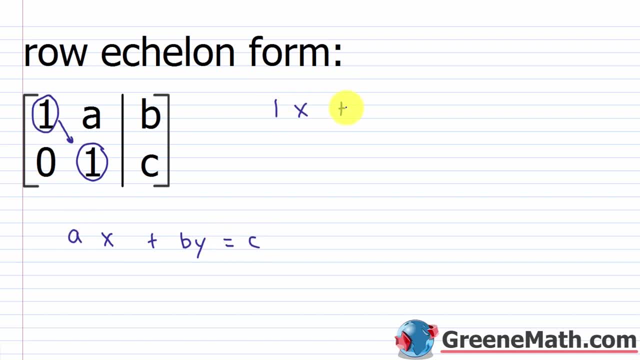 c. well, I know that I'd have one x plus ay is equal to b in this case, just using generic information, And I know here that I have zero x, so x is eliminated plus one y, or just y, equals c. 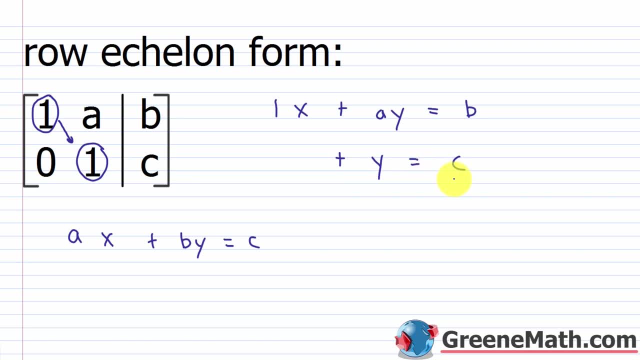 So from this, if I know y equals c, I can plug in for y here and I can find out what x is. Again, we're just taking the numerical information and finding our solution. So again, this is row echelon form. 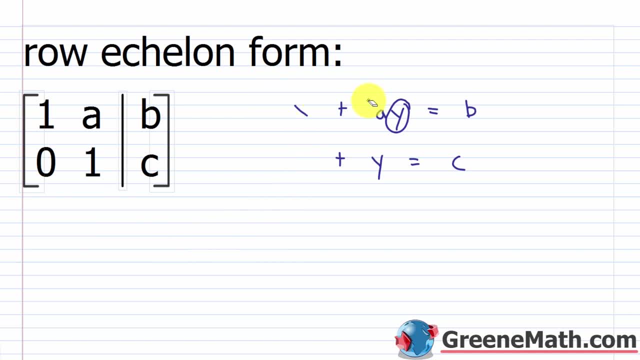 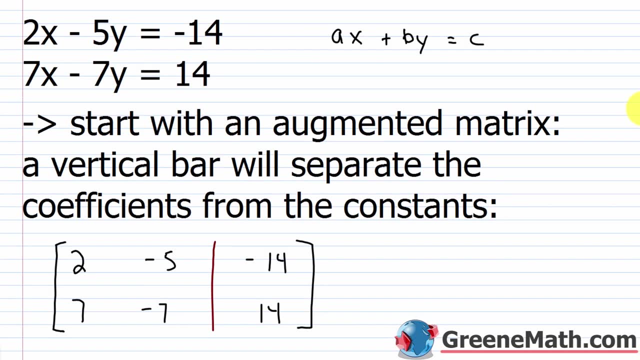 So I want you to write that down and then, once we get this down, I'm going to show you reduced row echelon form, which isn't any more complicated. All right, so I want to return now to the system that we were starting with. 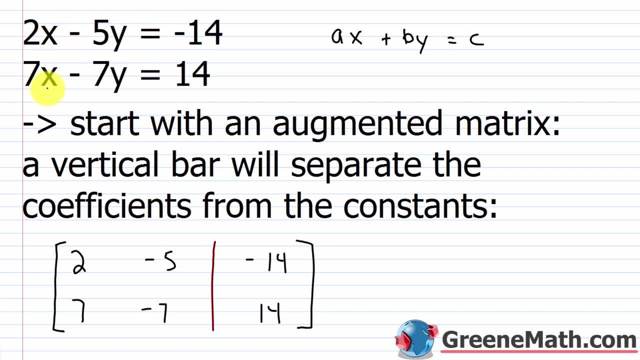 So again, it's 2x minus 5y equals negative 14.. It's 7x minus 7y equals 14.. So let's copy this information and we'll copy this and we'll bring it down to a new. 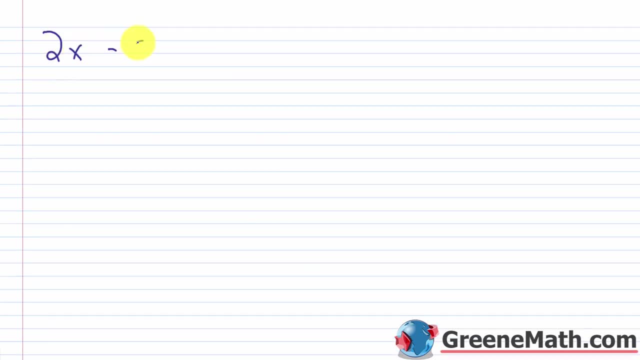 sheet of paper. So again we have 2x minus 5y equals negative 14.. We'll call this equation one. Then for equation two, we'll have 7x minus 7y equals 14.. All right, So again write the augmented matrix. 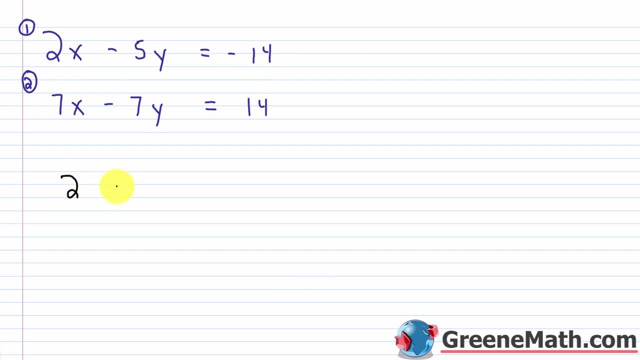 Just the numerical information. That's all we want. So we want 2,, we want negative 5, and we want negative 14.. We want 7,, we want negative 7, and we want 14.. A vertical bar will go right here to separate the coefficients from the constants. 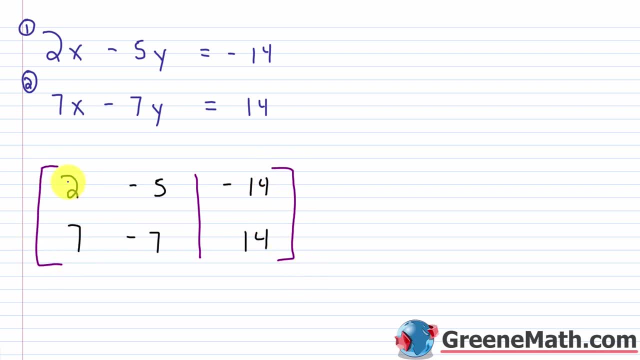 And our goal is what? Again, I want ones down the diagonal. So I want this to be a 1, and I want this to be a 1.. So down the diagonal. Okay, That's going to be a 1.. 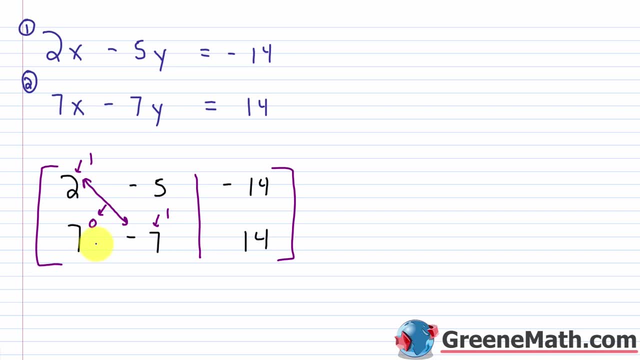 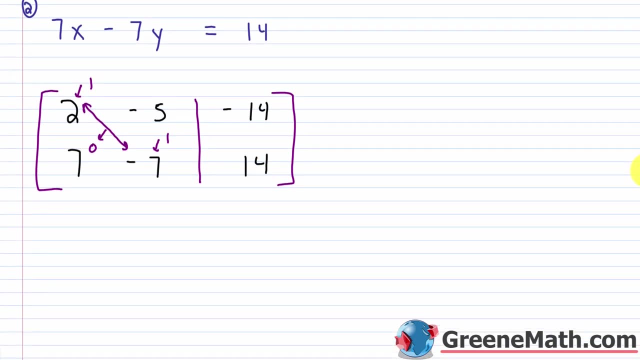 All right Beneath the diagonal, I want a 0.. And then these numbers here would be real numbers. So how do we achieve that goal? Well, again, we're going to use our row operations. So how could I make 2 a 1 using the row operations? 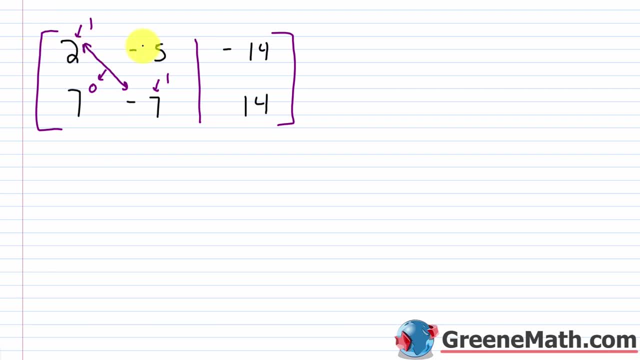 Well, I could simply multiply every number in this row by 1 half. 2 times 1 half equals 1.. So if I do that, what would I get? 2 times 1 half equals 1.. Negative 1 half again is 1.. 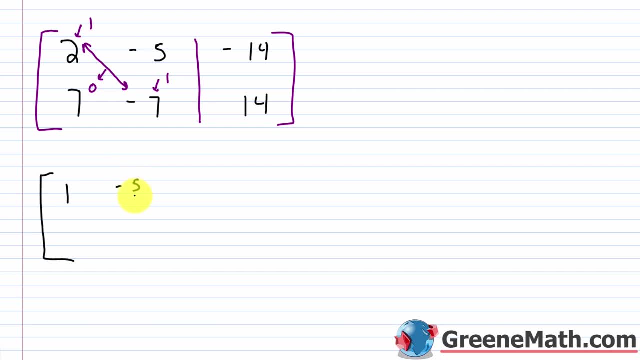 Negative 5 times 1 half is negative 5 halves, And negative 14 times 1 half is going to be negative 7.. Now for this one, I have 7, negative 7, and 14.. I haven't done anything there. 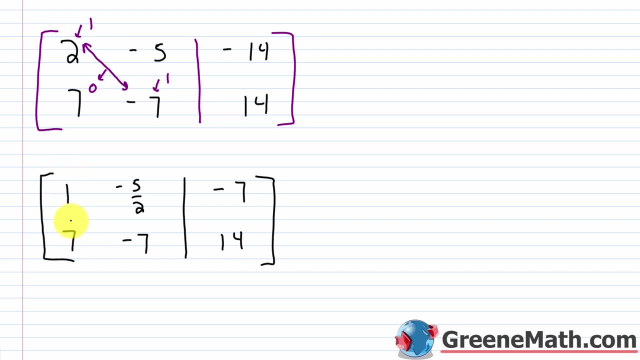 Okay. So now that we have this as a 1,, we want to make 7 into a 0.. It's best to work a column at a time, So starting here and working down. If I wanted 7 to be a 0,, what could I do? 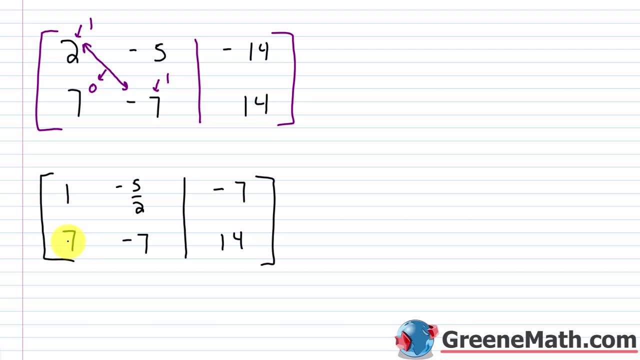 Well, I could multiply 7 by 0, but that's not going to work right. We can't multiply both sides of an equation by 0 and maintain the same solution. That's a violation. So what I have to do is I have to multiply this row here by something and add it to this. 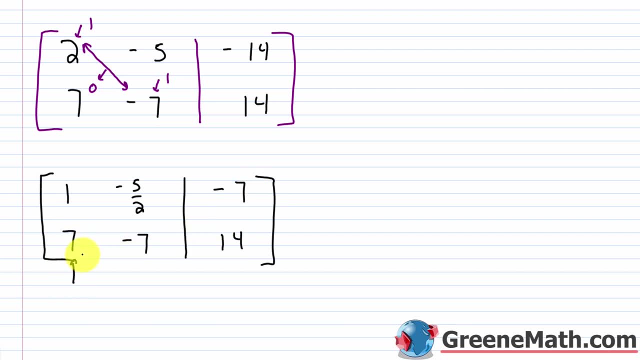 to get this to be 0.. So, first and foremost, what can I add to 7 to make it 0?? Well, obviously, negative 7.. So that means I need to multiply 1 by some value, And it needs to give me negative 7 so that, when I add it to 7, I get a value of 0. 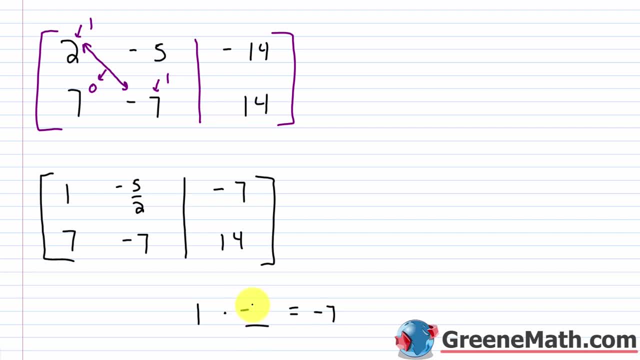 So, 1 times what would give me negative 7? 1 times negative 7.. So that means I'm going to multiply row 1 by negative 7.. And when I do that, what am I going to get? Well, 1 times negative 7 is negative 7.. 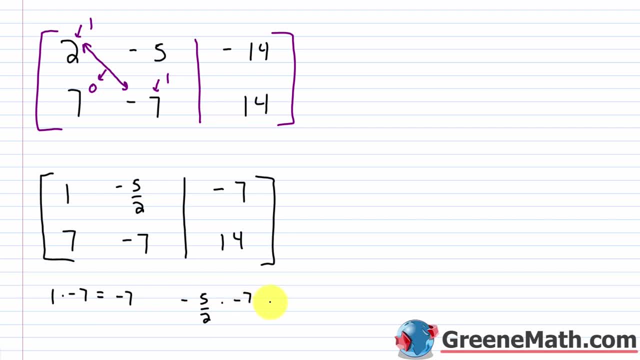 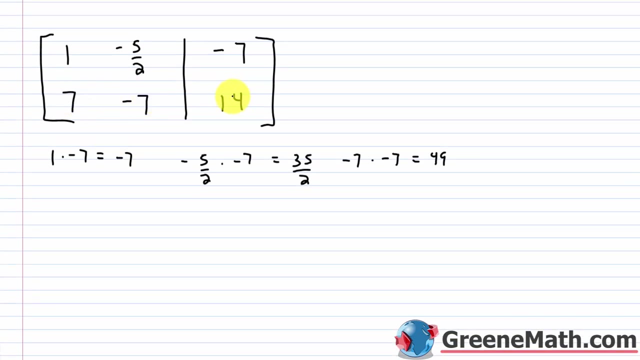 Negative 5 halves negative 5 halves times negative 7 would be 35 halves. And then negative 7 times negative 7 is going to be 49. So I'm going to take that information and I'm going to add it to each element here. 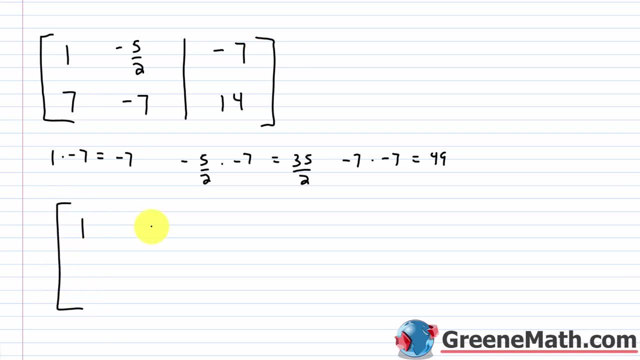 So this row 1, I'm just going to keep it the same, Remember I don't have to change it. Negative 7 plus 7 is 0. So 35 halves plus negative 7. So plus negative 7.. 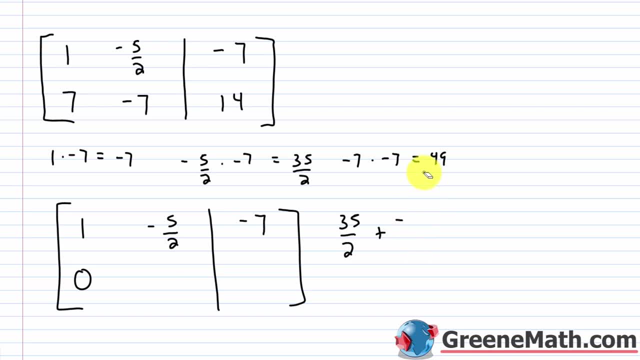 I multiply. I multiply this by 2 over 2.. That would be negative: 14 over 2.. And 35 minus 14 would give me 21.. So this is 21 halves, And then, lastly, I have 49 plus 14.. 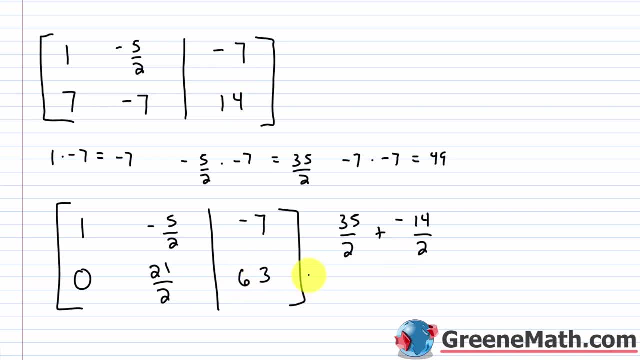 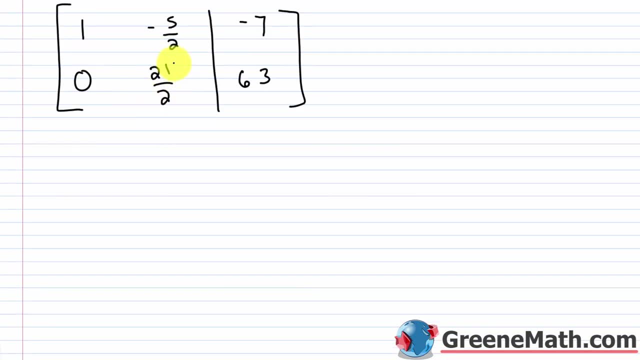 So 49 plus 14 would give me 63.. OK, So now let's scroll down The next thing I want to do, since I have a 1 here and a 0 here, remember, I want 1s down the diagonal. 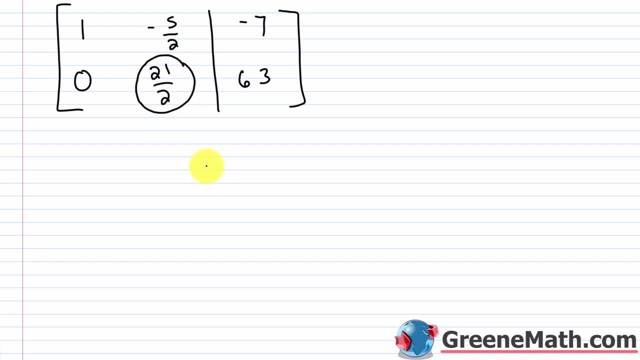 So how can I make this into a 1?? Well, that's easy. So I'm going to multiply this by 2 over 21, halves times the reciprocal, which would be 2 over 21,, would equal 1.. So just multiply row 2 by 2 over 21.. 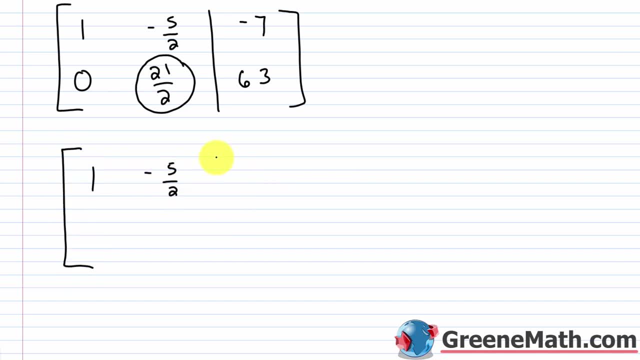 So multiplying 0 by anything is 0.. So let's just start out by saying this is 1, this is negative 5, halves this is negative 7.. So that's all the same: 0 again, times 2 over 21 is still 0. 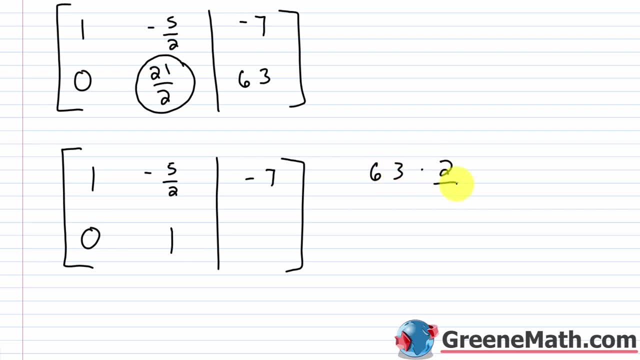 2 over 21 times 21 over 2 is 1.. So 2 over 21.. Well, 63 divided by 21 is 3.. So this cancels with this and gives me 3.. 3 times 2 is 6.. 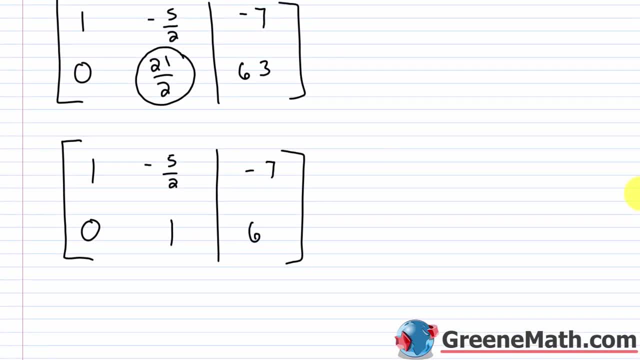 Now, what do I have here? Well, I have row echelon form, I have 1s down the diagonal, I have a 0 below And I have real numbers here, here and here. So once I'm in that format, I have enough information to get a solution. 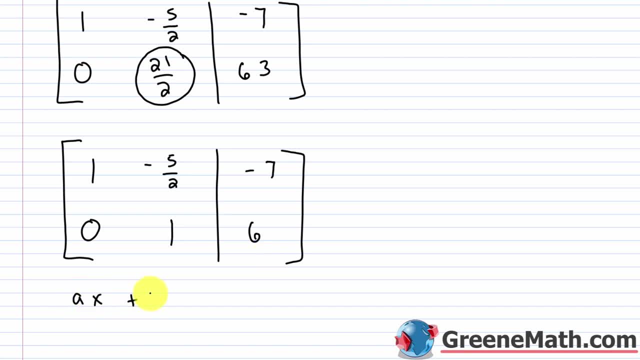 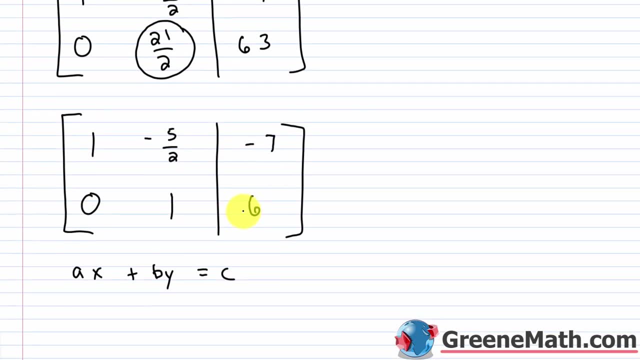 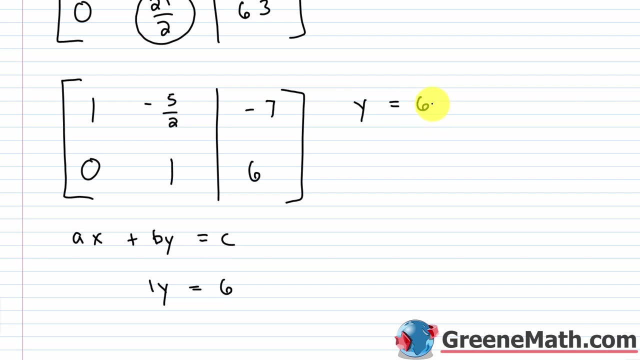 Remember this is ax plus by equals c, So forget about this top row. The bottom row is basically 1y is equal to 6.. So I know that y here is equal to 6.. Now I can take this information and plug it in here. 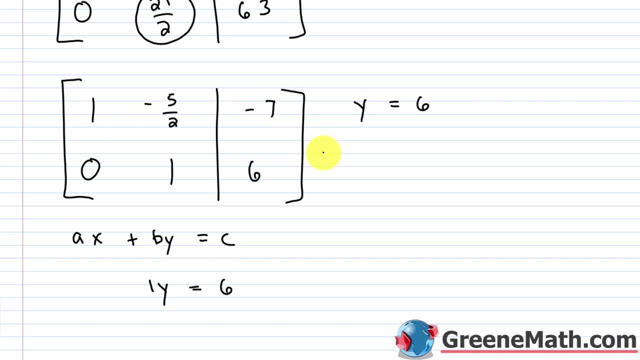 For this guy right here I have that 1x, or just x, plus negative 5, halves times y. y is 6, is equal to negative 7.. So I know, if I do a little bit of math here, 6 divided by 2 is 3.. 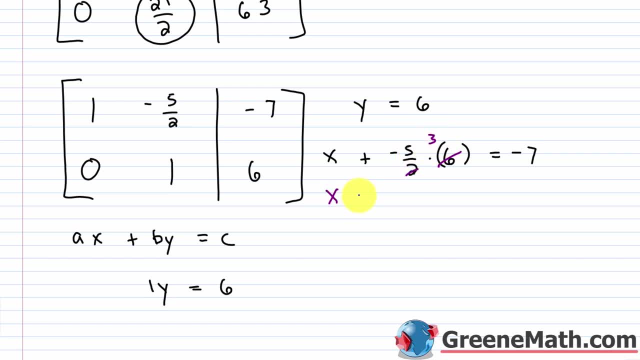 Negative 5 times 3 is negative 15.. So we would have: x minus 15 is equal to negative 7.. We would add 15 to each side of the equation And we would have that x is equal to 8.. So x equals 8,, y equals 6.. 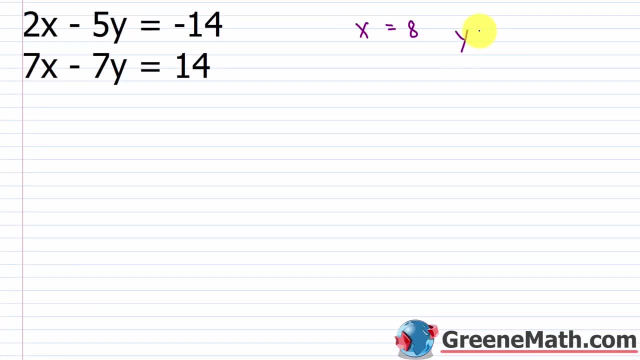 So I'm going to write that x equals 8, y equals 6.. We're the ordered pair, 8 comma 6.. Now let's check this real quick. I'm not going to check any in the future because of the interest of time. 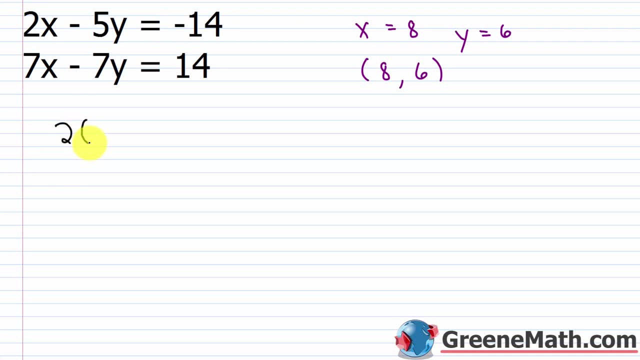 But I just want to show you that this works. So we have 2 times put in an 8 for x, minus 5 times plug in a 6 for y. This equals negative 14.. 2 times 8 is 16.. 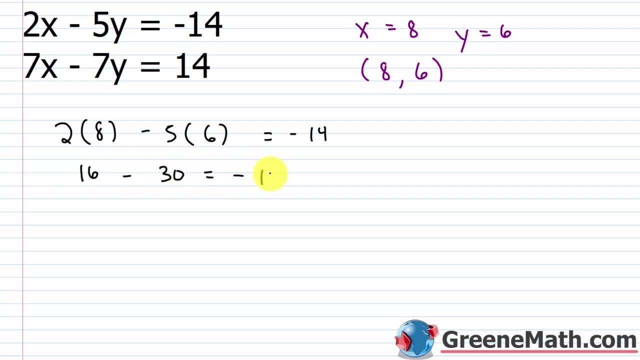 Minus 5 times 6 is 30. This should equal negative 14. And it does. 16 minus 30 is negative 14. So negative 14 equals negative 14. So it works out. here For the next equation of this system, we have what? 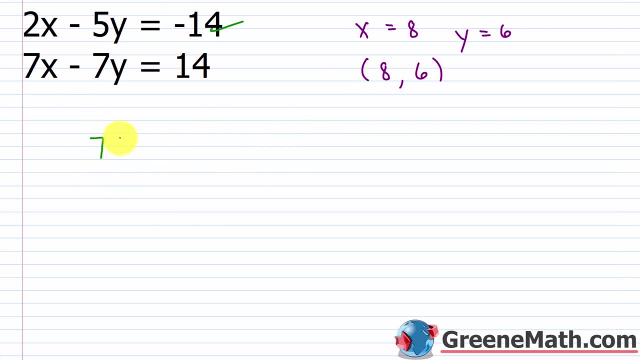 We have that 7x. so 7 times 8, minus 7y y is 6, equals 14.. 7 times 8 is 56, minus 7 times 6 is 42. Does that equal 14?? 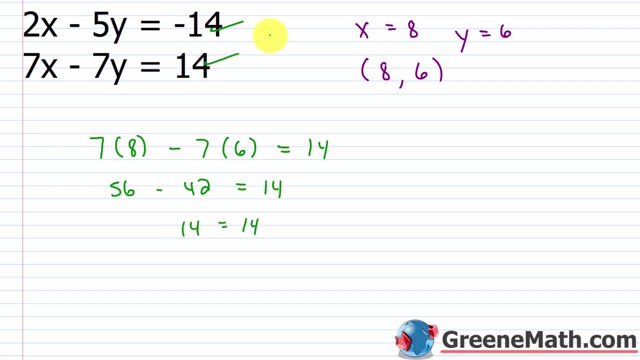 Yes, it does. We have 14 equals 14. So it works out here as well. So I know you might be a little confused on this. It's okay. It's something new, It's something that you just have to practice. 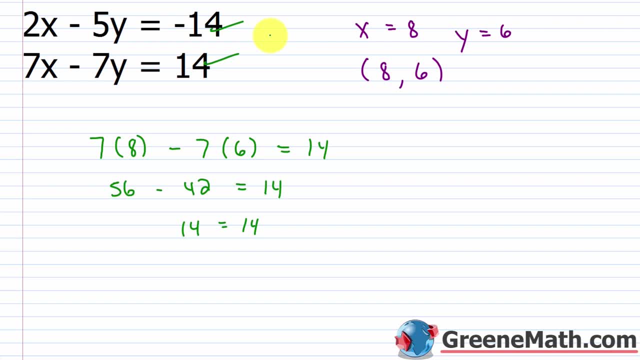 But hopefully you can see the concept and understand what we're doing. We're basically just taking the numerical information and we're using the elimination method, but we're doing it in a more compact way. So let's take a look at the next example. 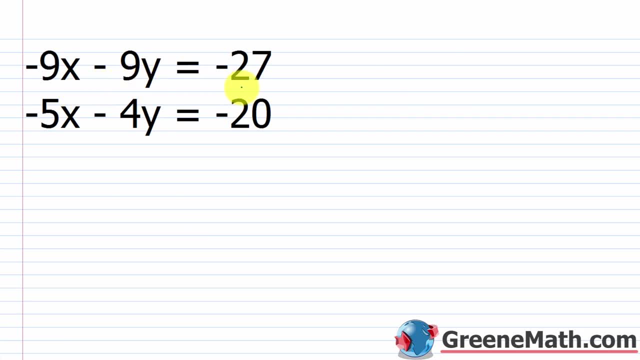 So we have negative 9x minus 9y equals negative 27.. We have negative 5x minus 4y equals negative 20.. So again I'm going to take the numerical information here. So a negative 9,, another negative 9, and a negative 27.. 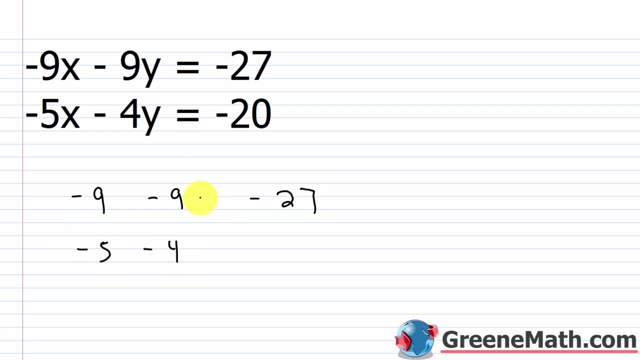 I have a negative 5, a negative 4, and a negative 20.. And again, you want to make sure that these equations are written in standard form: ax plus by equals c, Both of them on top of each other. Verify that the x's are in the same place. 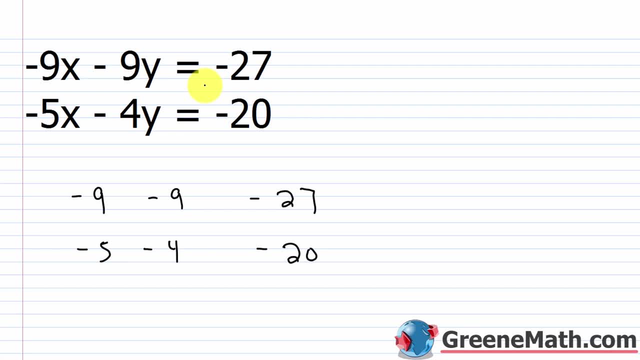 the y's are in the same place, the coefficients are in the same place, so that your information is correct. So you have your vertical bar, okay, that separates the coefficients from the constants, And so we have our equation, We have our augmented matrix. 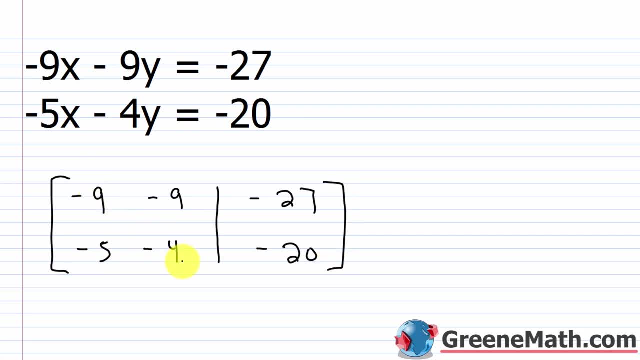 All right. so remember, we want 1s down the diagonal, okay, so we want this to be a 1, and we want this to be a 1, and we want a 0 below, and then these can be real numbers. 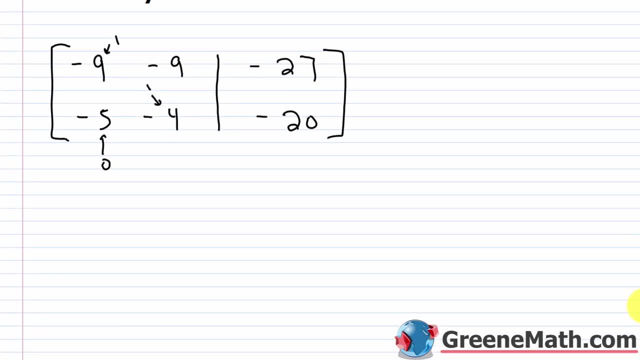 All right, so let's get started. How would I make negative 9 into a 1 using the row operations? Well, that's easy. I can always multiply negative 9 by the reciprocal, which is negative 1- 9th. 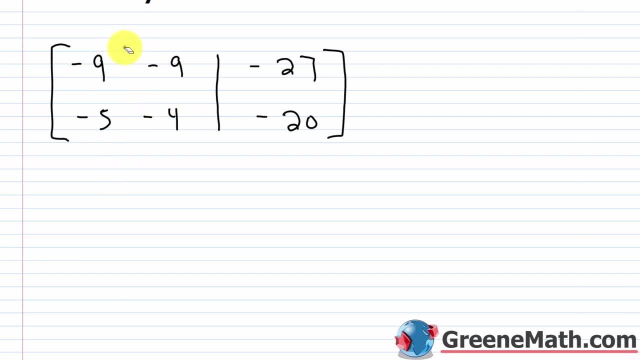 If I multiply negative 9 by negative 1- 9th, I know that this would be 1.. If I multiply negative 9 by negative 1 9th, again I'm going to get a 1.. If I multiply negative 27 by negative 1: 9th: 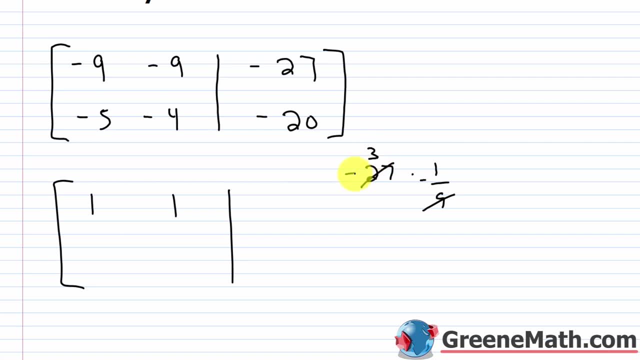 this cancels with this and I get a 3 here. So negative 3 times negative, 1 would be 3.. And then now I have this row: negative 5, negative 4, and negative 20.. All right, so now I want this next guy here. 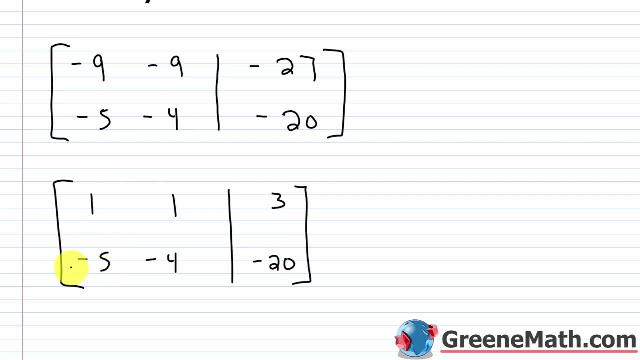 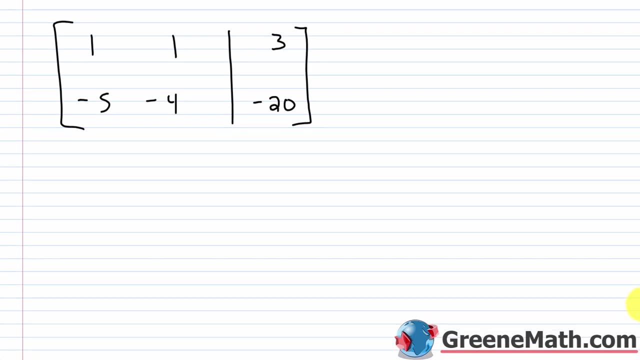 negative 5,. remember, I work a column at a time, so I want this to be a 0. So what can I do? Well, again, I want to add something to negative 5 to give me 0.. Well, I know, negative 5 plus 5 would give me 0,. 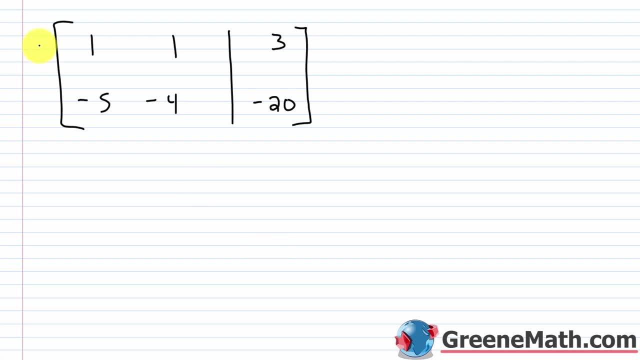 so in order to do that, I would multiply the first row here by 5, right, because 1 times 5 would give me 5.. So I multiply the first row. 1 times 5 would equal 5,. 1 times 5 would again equal 5,. 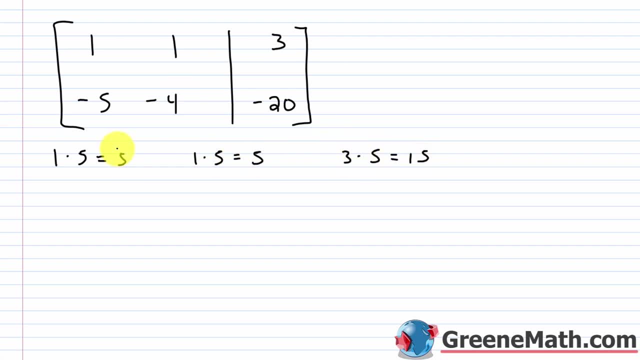 and then 3 times 5 would be 15.. So I'm going to take these results here and add them. So my first row I'm just going to keep it the same: 1,, 1, and 3.. So 5 plus negative 5 is 0,. 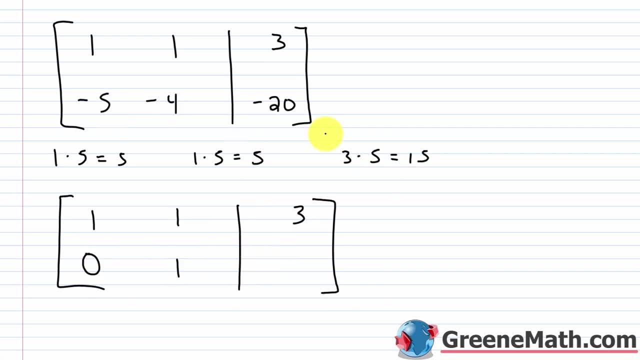 5 plus negative 4 is 1, and then 15 plus negative 20 is negative 5.. Now it just so happens that this is an easy example, and I've already got what I want, which is row echelon form. 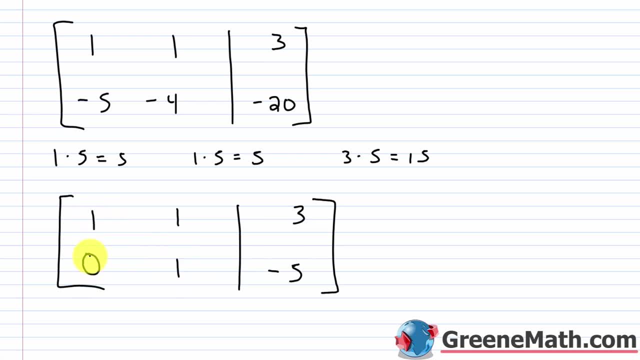 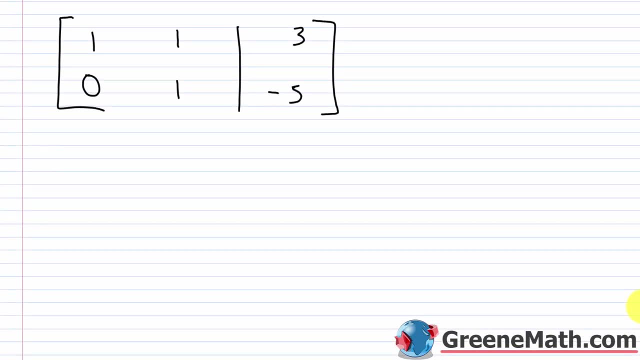 I've got 1s down the diagonal, I've got a 0 over here and I've got real numbers here. So again, once we have it in this format, we can use substitution to find our solution. So I know that from this bottom row here. 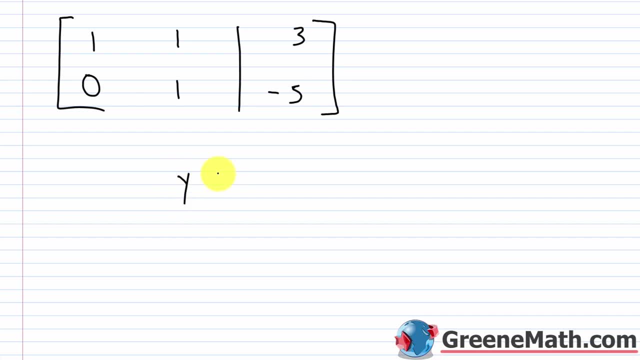 I would have 1y or just y is equal to negative 5.. In the top part here I have that x plus y, because I have 1x plus 1y is equal to 3. So just plug in a negative 5 here. 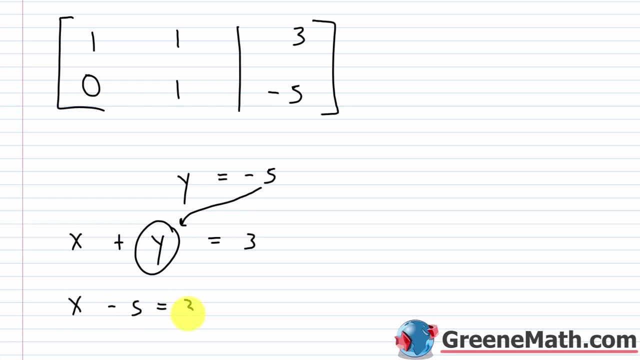 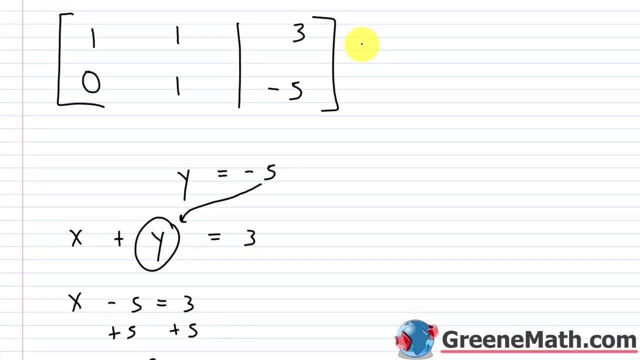 and you'd find that x minus 5 equals 3.. Add 5 to each side of the equation and you're going to get that x is equal to 8.. So the solution for this system would be that x is equal to 8,. 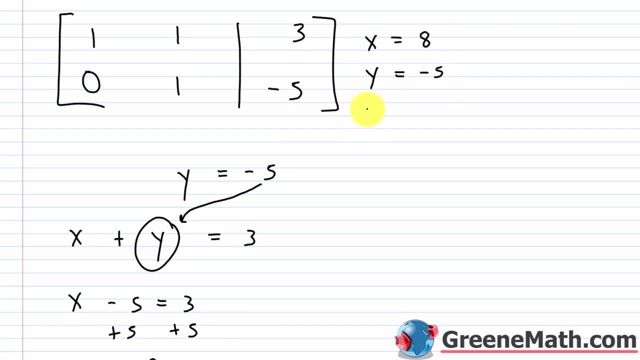 y is equal to negative 5.. Or as an ordered pair, you could say 8, negative 5. And you can pause the video, go back to the system and check it And verify that it's the correct solution. I've already done that. 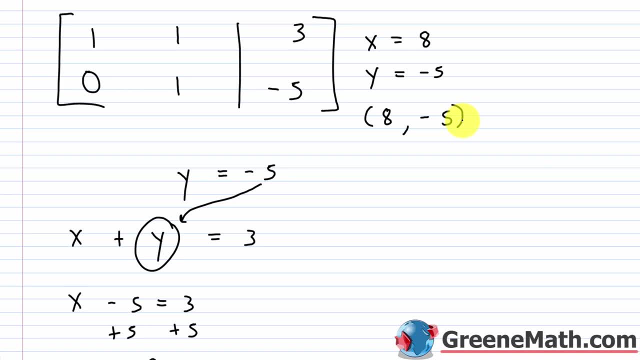 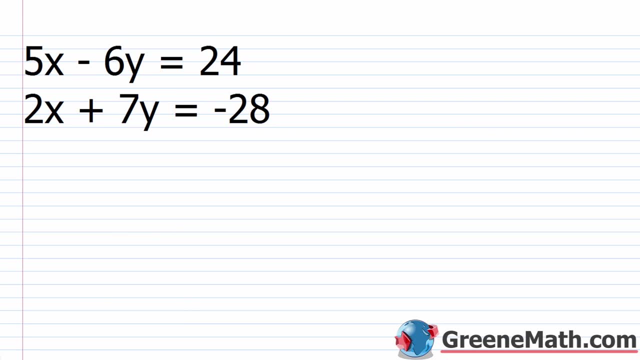 so I know that 8, negative 5 is the solution. Alright, let's take a look at one more example And what I'm going to do. in this example. I'm going to show you reduced row echelon form as well as row echelon form. 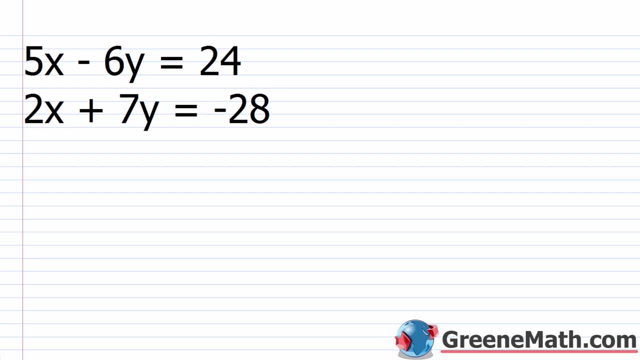 And I'm going to explain the difference between the two. So we have 5x minus 6y equals 24.. We have 2x plus 7y equals negative 28. So again, ax plus by equals c. So you make sure your equations are in that format. 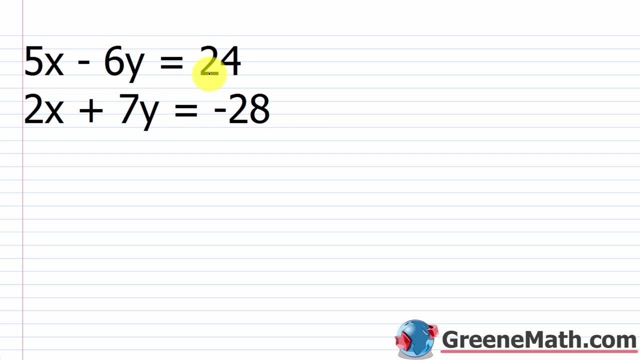 Again, a lot of textbook examples are going to jamble things up, so it's not in that format. You've got to write it that way, so your information is consistent. Alright, so I have a 5,, a negative 6,. 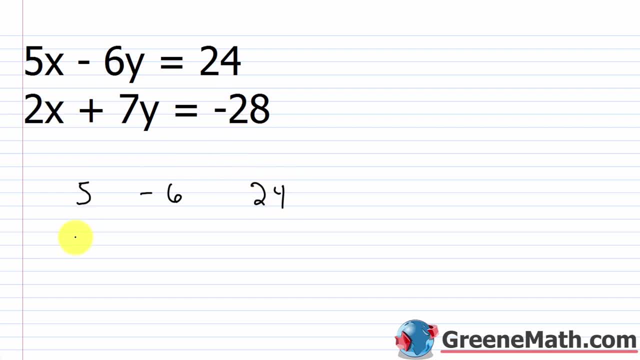 and a 24.. The information here: I have a 2,, I have a 7, and I have a negative 28. So I have my vertical bar that separates the two, the coefficients, from the constants. And now we get to work. 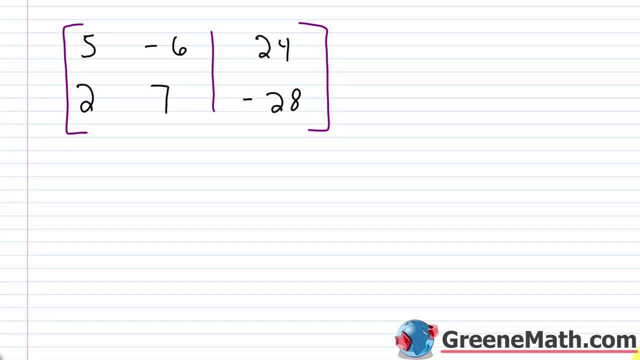 So again we're going to talk about row echelon form first. So that's ones down the diagonal, a zero over here and real numbers here. So let's start with the first column here. How can I make 5 into a 1?? 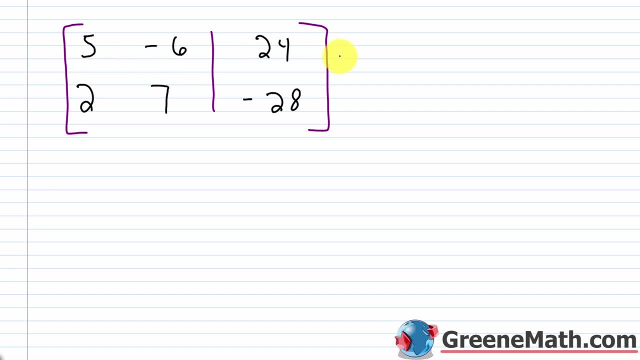 Well, I can multiply row 1 by 1 fifth. 5 times its reciprocal of 1 fifth gives us 1.. So if I multiply 5 times a fifth, I get 1.. If I multiply negative 6 by a fifth, 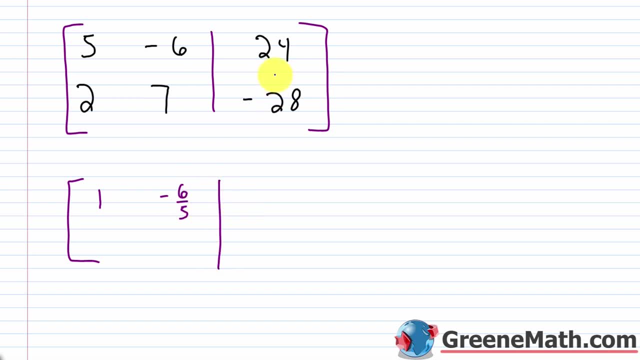 I get negative 6 fifths. If I multiply 24 by a fifth, I get 24 fifths, And then row 2 stays the same for now. So 2, 7, and negative 28.. Okay, so let's scroll down. 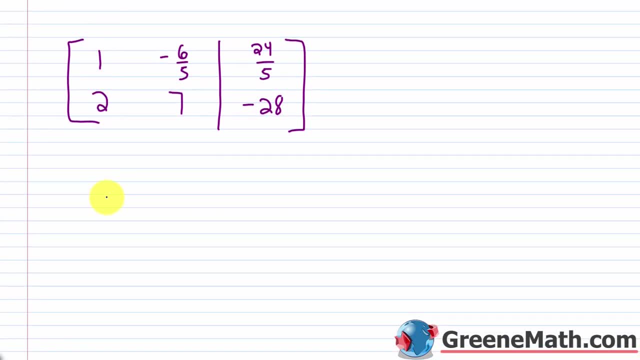 Now again, working at a column at a time, how can I make 2 into a zero? Well, I think about row 1 here. To get 2 into a zero, I've got to add 2 to its opposite. 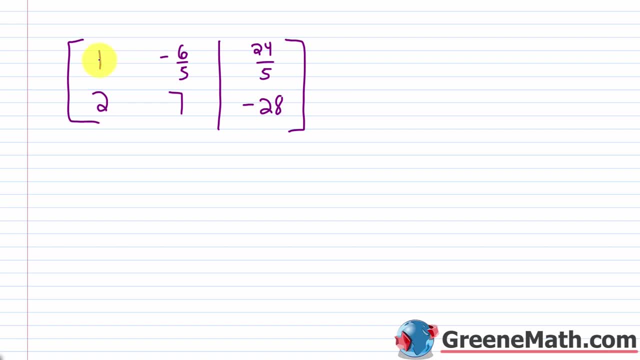 which is negative 2.. So what can I multiply 1 by to get a result of negative 2?? Well, of course, just negative 2.. So if I multiply row 1 by negative 2, 1 times negative 2 gives me negative 2.. 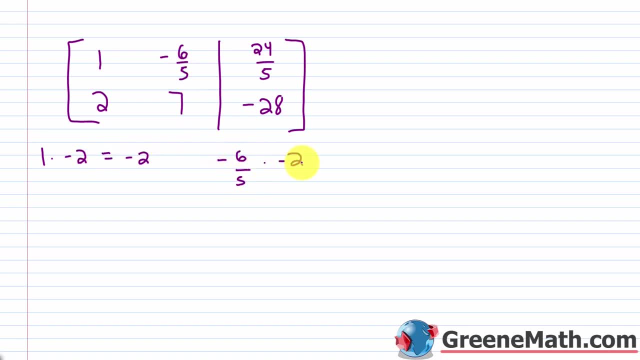 Negative: 6 fifths times negative 2.. I know the negatives would cancel. You'd basically have 12 fifths And then 24 fifths. 24 fifths times negative. 2 would be negative 48 fifths. So this is negative 48 fifths. 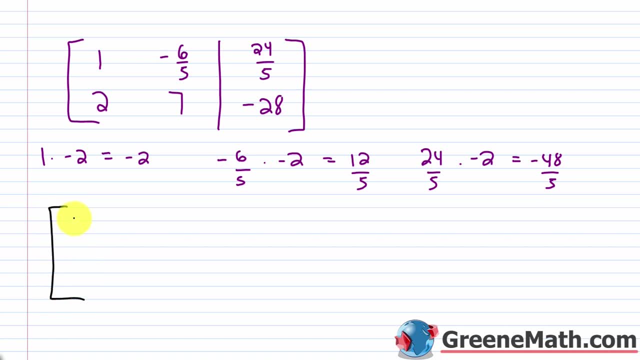 So for row 1, I'm keeping that the same, So a 1, a negative 6 fifths and then a 24 fifths. For row 2, I'm going to take the result that I got and I'm going to add: 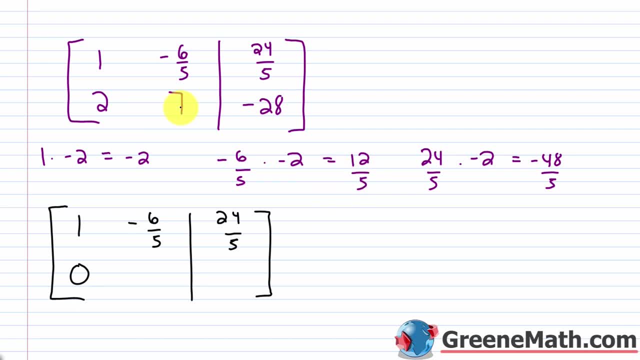 So negative 2 plus 2 is 0.. I'm going to have 12 fifths plus 7.. So 12 fifths plus 7.. I could write that as 35 fifths. 12 plus 35 is 47.. 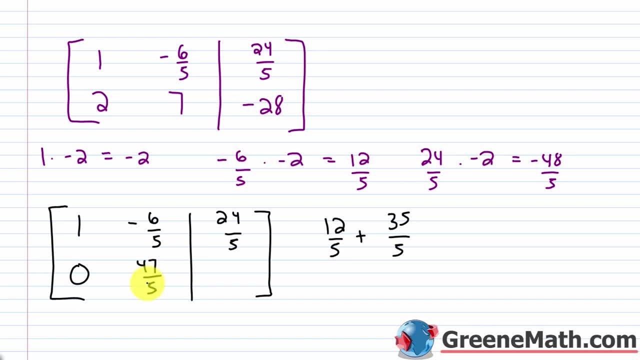 And then the common denominator of 5 is what that's going to be over. So that's 47 fifths. And then, if we think about the next result, you'd have negative 48 fifths plus negative 28.. So negative 48 fifths plus. 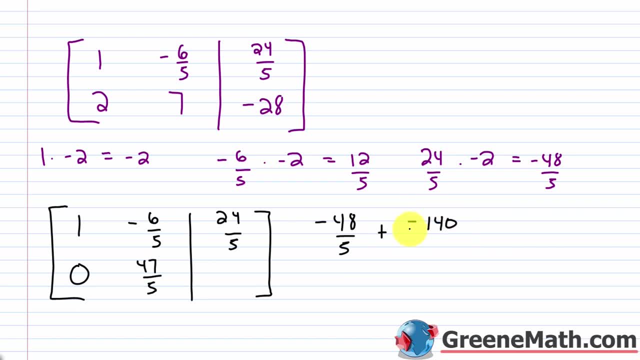 Negative 28 times 5 is negative 140. So I'd have negative 140 over 5.. So if I add these two together- negative 48 plus negative 140, that would give me negative 188.. So I'd have negative 188 over 5.. 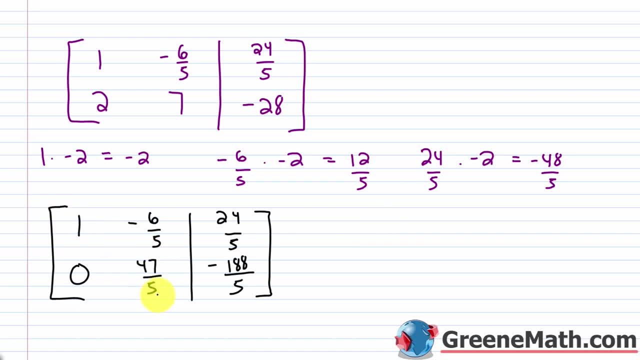 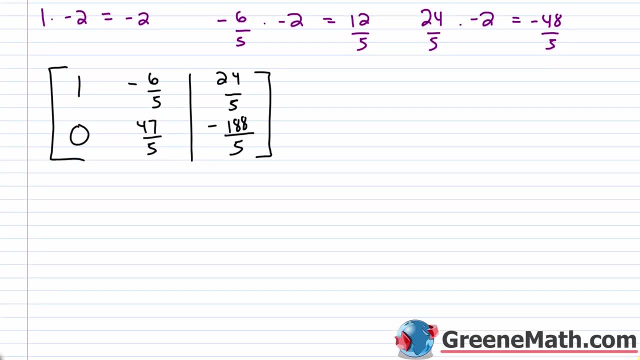 All right, So the next thing I want to do is make this a 1.. I want 1s down the diagonal 0 below. I've already got this part. I just need this part, So let's scroll down here. 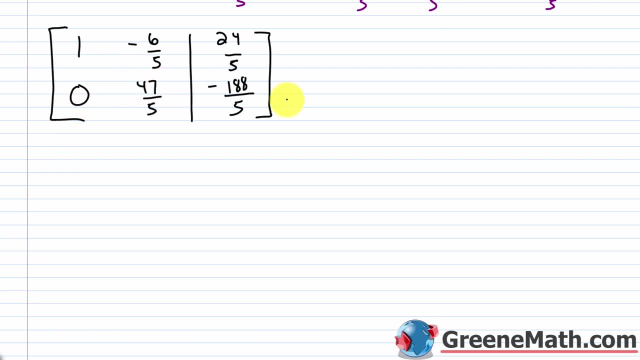 And it's very easy: I just multiply row 2 by the reciprocal of 47 fifths, which is 5- 47ths. So let's keep row 1 the same. So row 1 stays the same, A 1, a negative 6 fifths and a 24 fifths. 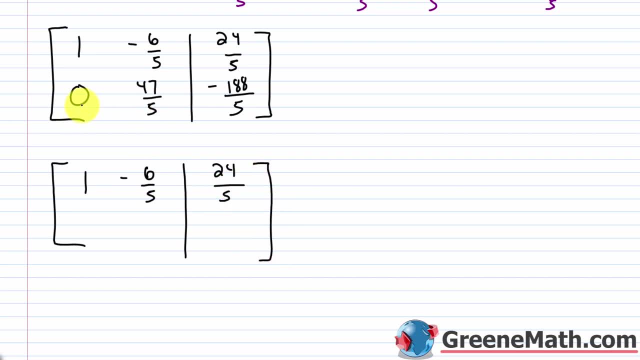 For row 2, again, if I multiply 5 over 47 by 0,, I get 0.. 5 over 47 times 47 over 5 is 1.. And then 5 over 47 times negative, 188 over 5.. 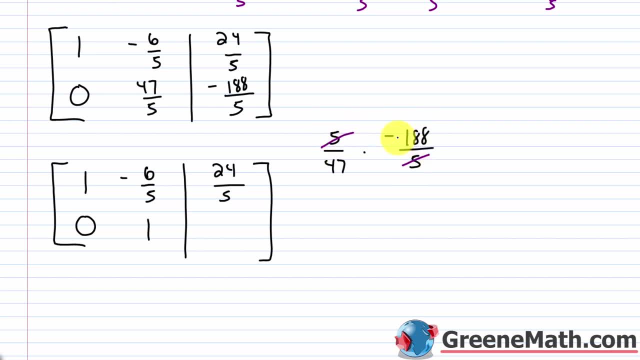 Well, I know the 5s would cancel And negative 188 divided by 47 is actually negative 4.. So at this point I have enough information to get a solution. I know that y is equal to negative 4.. All right, 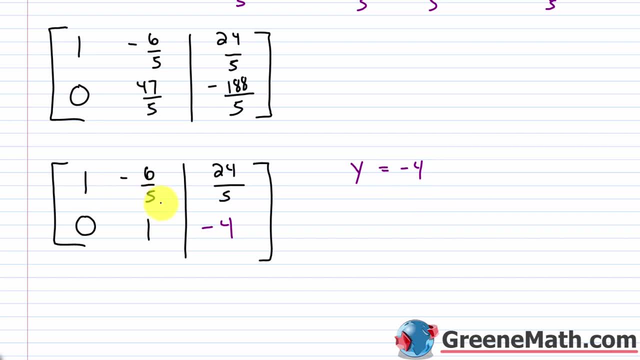 So if y equals negative 4, I can plug in for y in this part. So I would have x minus 6 fifths. y is equal to 24 fifths. Scroll down a little bit And again y is negative 4.. 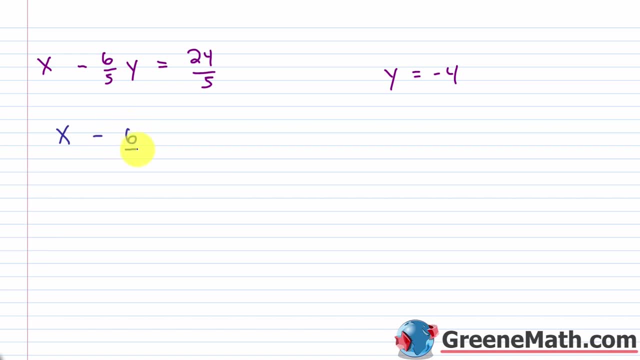 So what we're going to get is that x minus 6 fifths times negative, 4 is equal to 24 fifths. So we know negative times negative is positive. So you get x plus 6 times 4 is 24.. So fifths equals 24 fifths. 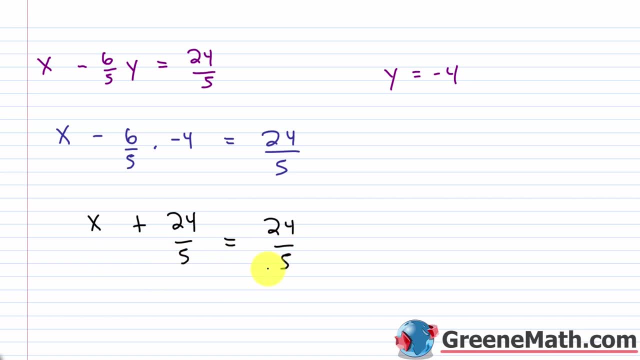 So we know x has to be 0, right? If I subtract 24 fifths away from each side of the equation, we would get x is equal to 0. So y equals negative 4, x equals 0. So you can pause the video, check and make sure. 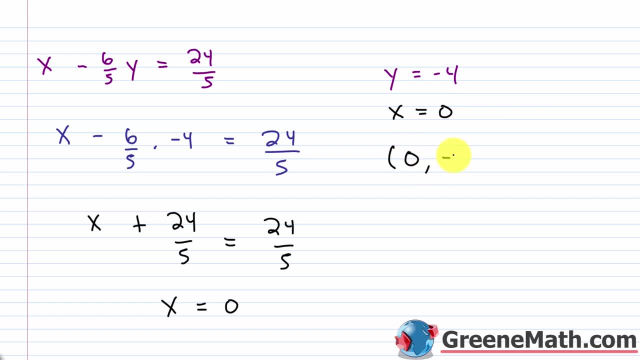 that's the correct solution. The ordered pair is 0 comma negative 4.. Now I want to talk about reduced row echelon form. So we're going to go back to the row echelon diagram. I gave you All right. So we know at this point that row echelon form 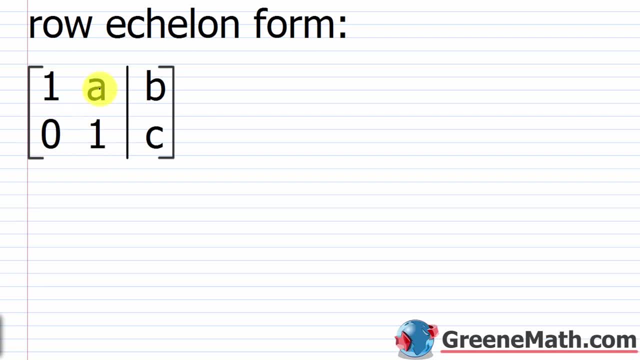 is ones down the diagonal, a, 0 below, and you have real numbers a, b and c. So with this form we have the information to go back and plug into the system and get our solution, But with reduced row. echelon form. 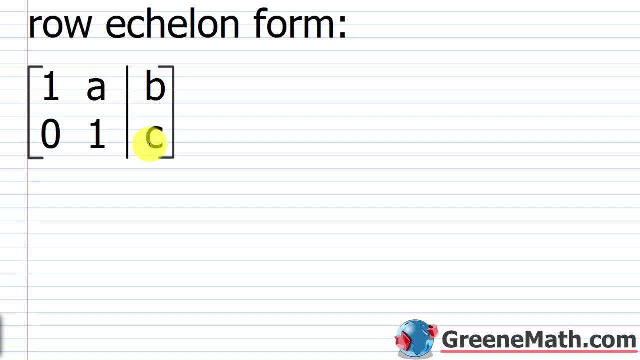 we don't have to go back and plug things in. We have our solutions. Let me show you that This is called reduced row echelon form, So I would have ones down the diagonal still. So this is a 1 and this is a 1.. 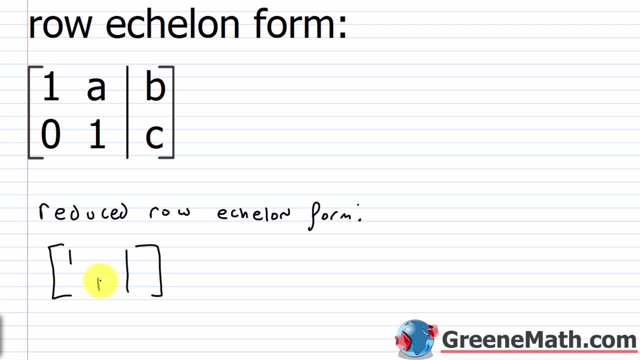 But everything in terms of the coefficients other than down the diagonal is going to be a 0. So it's a 0 here and a 0 here, And then you have two real numbers here on the right side of your vertical bar. So let's just say this is a and this is b. 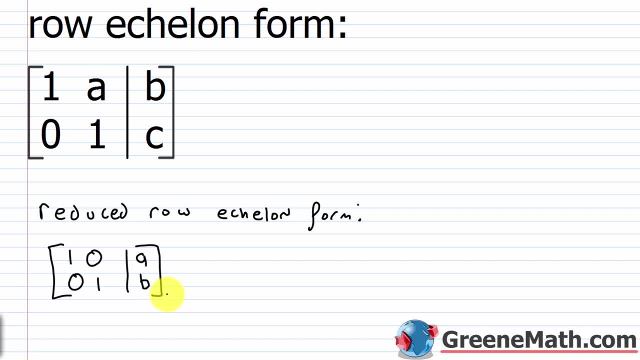 So with this guy right here I don't need to use substitution, because I know that 1x or just x is equal to a, So x equals a, And then 1y or just y is equal to b. So I have my solution in this form. 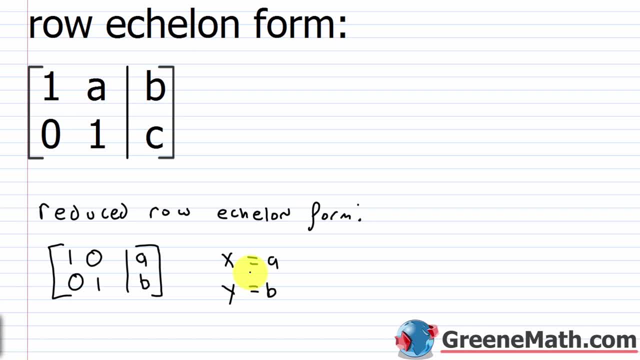 without going back to plug things in. So you might ask the question: which one is faster? Well, generally reduced row echelon form is going to be a little bit quicker because we don't have to go back and plug things in. We have x equals something, y equals something. 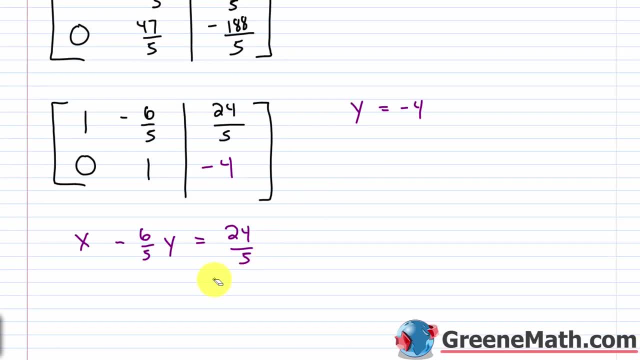 So I want to just show you on that last example. So this is where we kind of stopped and used substitution, So let's pretend that we could have continued. So let me just copy this and bring it to a fresh sheet. So we already know: y equals negative, 4x equals 0.. 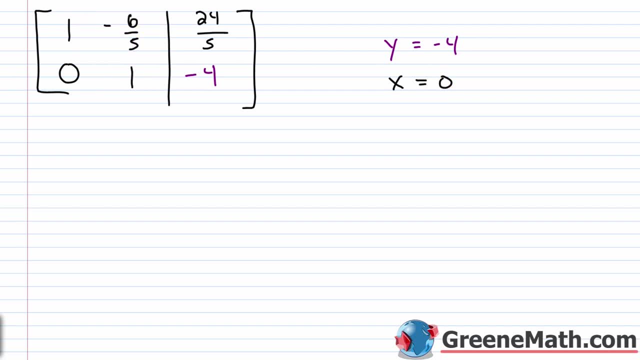 In order to get that information, I want to make this part right here, this part right here, into a 0.. I already know that y is negative 4.. I've got that information, But I want to know x is equal to 1.. 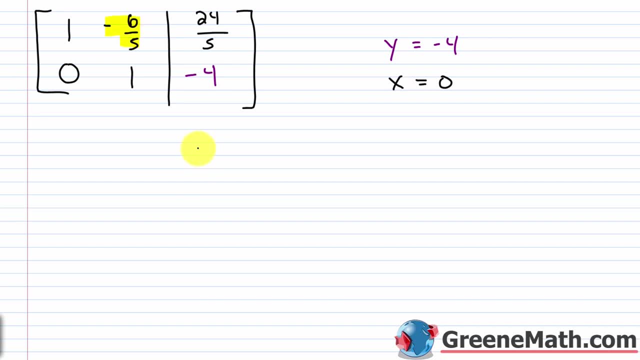 So how could I make this into a 0?? Well, you've got to think about what I could add to negative 6 fifths to get to 0.. Negative 6 fifths plus what- This is easy 6 fifths equals 0.. 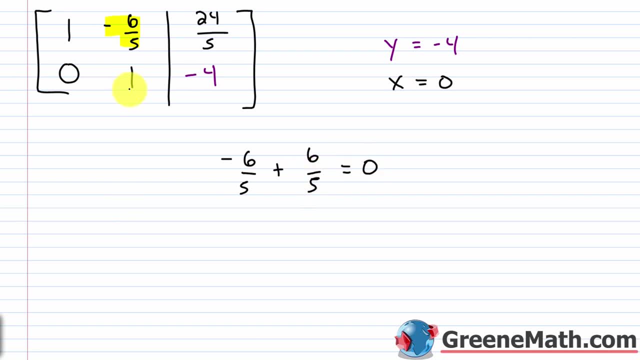 Well, since this is a 1, I just need to multiply this by 6 fifths. So if I multiply row 2 by 6 fifths and add it to row 1, I'm going to get what I need. So let's set this up here. 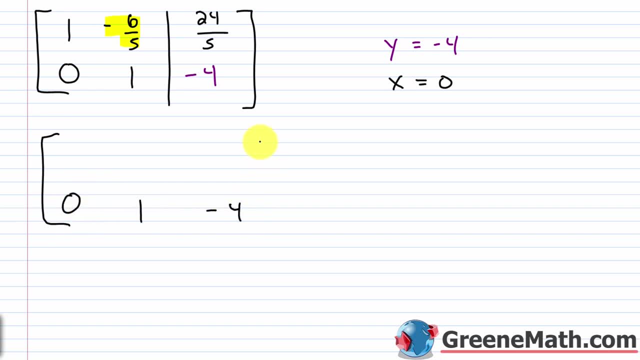 So let's set up row 2 as 0, 1, and negative 4.. So that's already there. 0 times 6 fifths is 0.. 0 plus 1 is 1.. 1 times 6 fifths is 6 fifths. 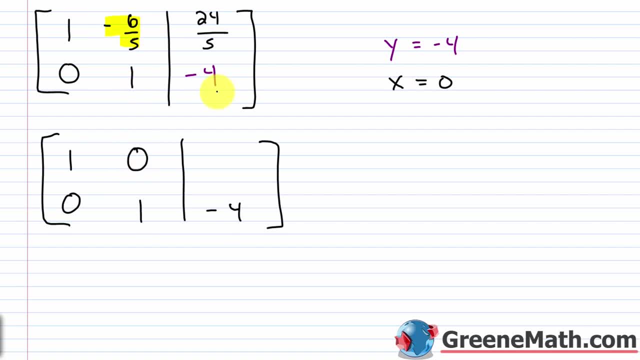 6 fifths plus negative 6 fifths is 0.. Negative 4 times 6 fifths. So negative 4 times 6 fifths. Negative 4 times 6 is going to give me negative 24.. So I'd have negative 24 fifths. 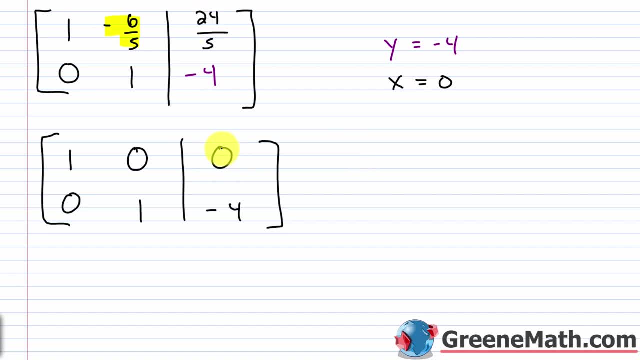 Now negative 24 fifths plus 24 fifths is 0.. So what did I find here? now? I found that x is equal to 0,, which is what it is. y is equal to negative 4,, which is what it is. 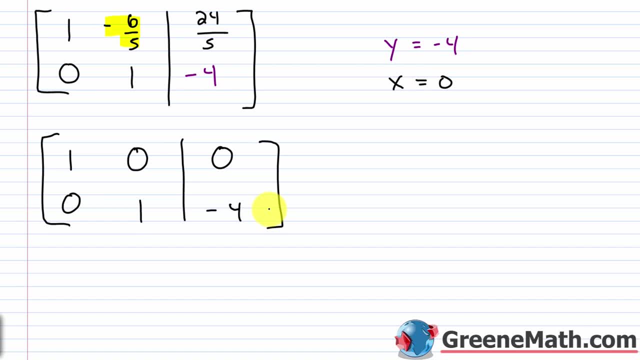 So with this form I don't need to go back and plug things in, So in most cases it's just a little bit quicker. But I want you to understand both forms because you might get tested on them. So you have row echelon form. 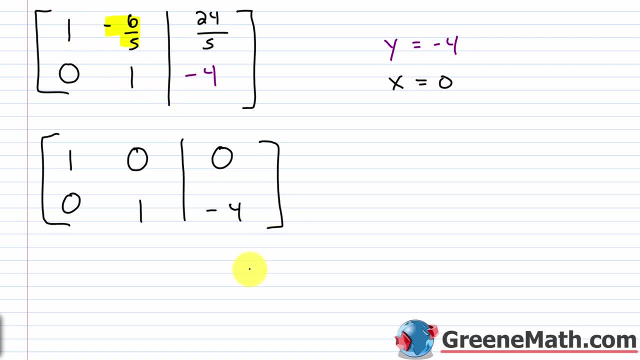 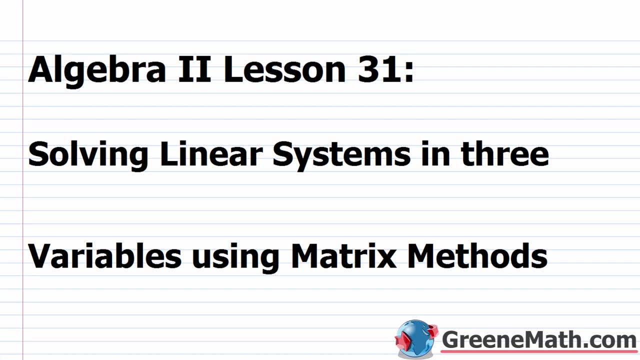 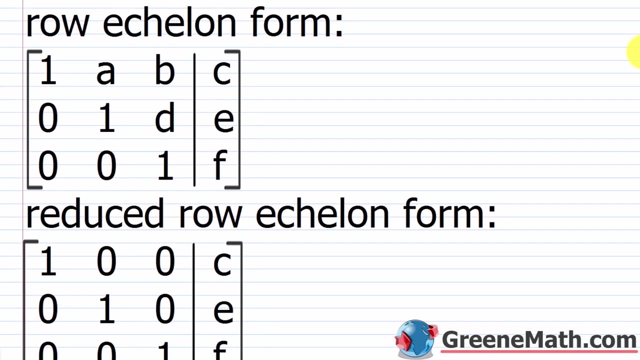 which is this. And you have reduced row echelon form, which is this. Hello and welcome to Algebra 2, Lesson 31.. In this video, we're going to learn about solving linear systems in three variables using matrix methods. So in the last lesson, 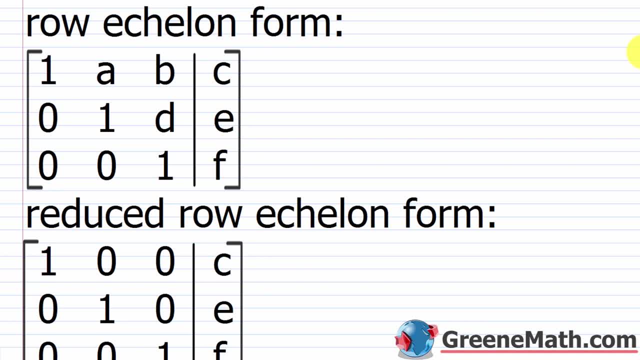 we learned how to use an augmented matrix to solve a linear system in two variables. In this lesson, we're going to push ourselves one step further And we're going to work with linear systems in three variables. So I want you to recall that our goal 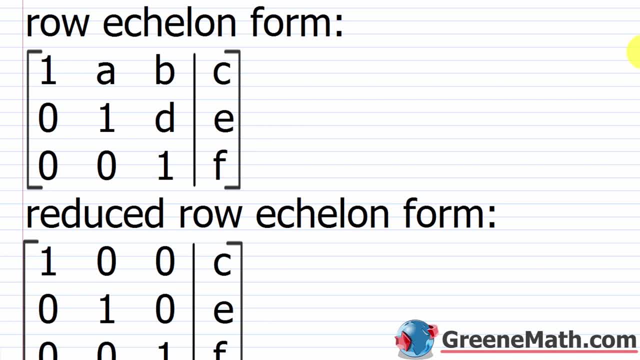 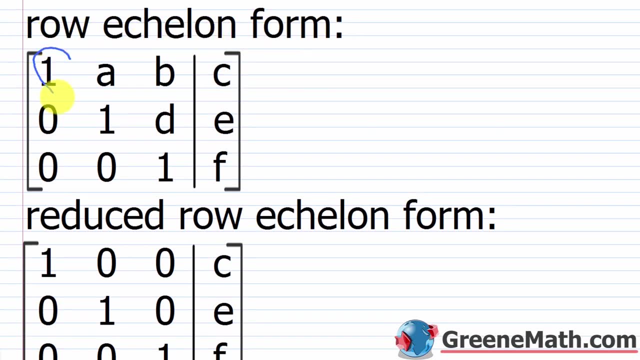 is to transform our augmented matrix, which is nothing more than the numerical information from the system, into a matrix that looks like either this one or this one. So the top one is known as row echelon form. So we have ones down the diagonal. 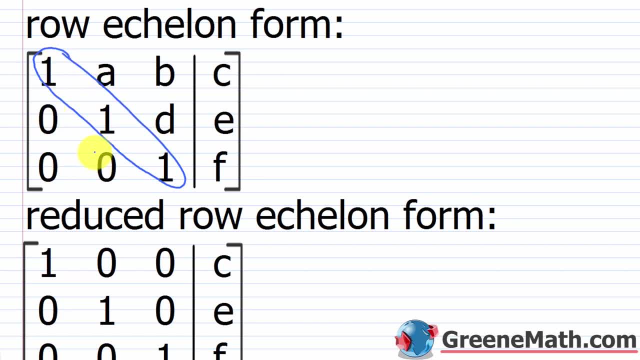 and we have zeros below. So you might say: well, how do I go about getting a solution from this information? Well, I want you to recall that you want to write each equation in standard form before you input the numerical information. So I usually would say: 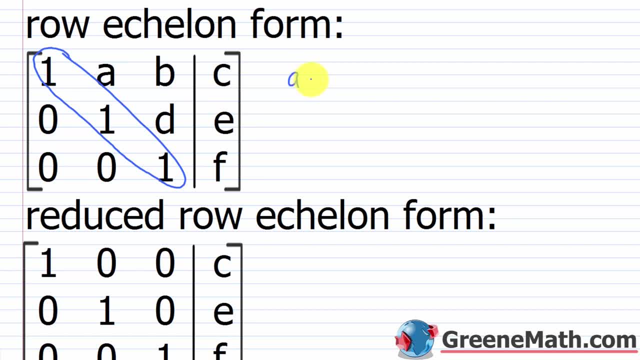 for a linear system in three variables. we want to do ax plus by plus cz equals d, Where a is the coefficient for x, b is the coefficient for y, c is the coefficient for z and d is just a constant. So we have our column with coefficients for x. 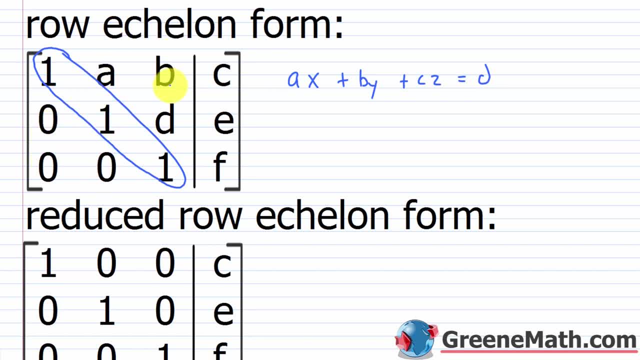 a column with coefficients for y, a column with coefficients for z and then constants. So very easy to understand where the information goes. Now, if I know that this is zero, and this is zero, that means that x and y are eliminated in this row. 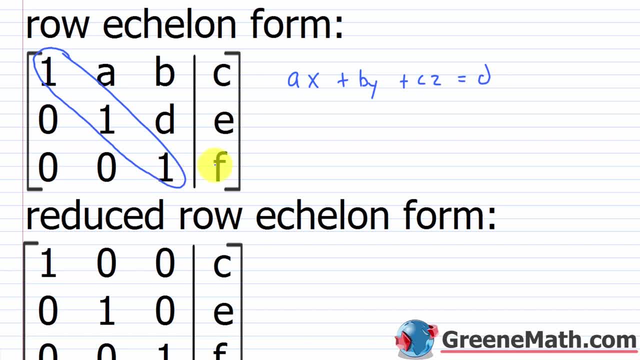 So then I have one z, or just z is equal to some real number, f. Using that information, I can go plug into this row here, because this corresponds to x being eliminated and only having y and z, If I know what z is. 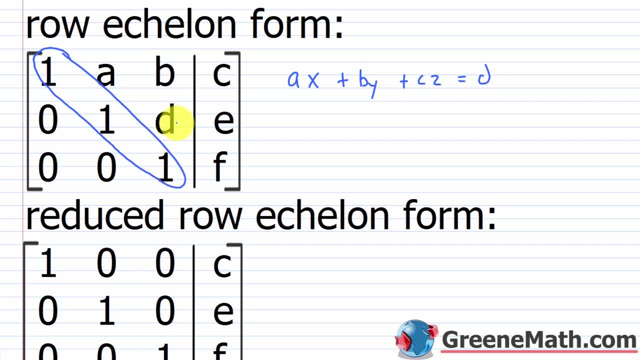 then it's a piece of cake. I can just solve for y. Once I now have y and z, I can go into the top row and figure out what is x Now, if you don't want to go through all that work with the substitution. 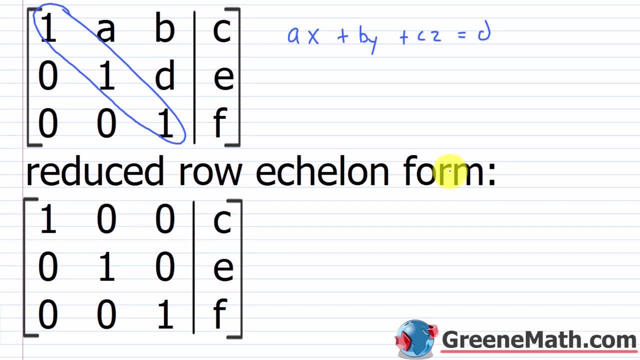 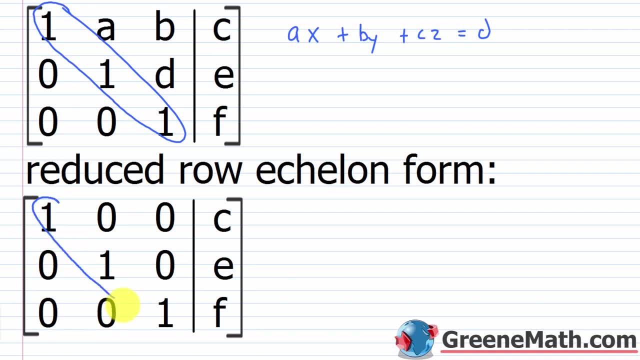 you can use reduced row echelon form. With this form you don't need to do anything other than look at your matrix to get the solution for the system. You have ones down the diagonal. You have zeros above and below, So I can simply look at this and say: 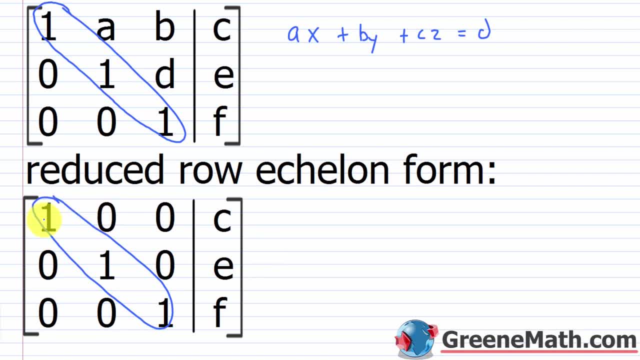 okay. well, y and z are eliminated here. X is some real number c, Y is some real number e, Z is some real number f. So in each row you'd have a solution for one of the variables. So again with this form: 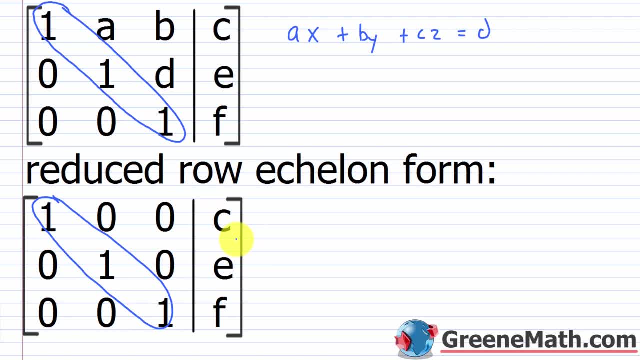 you don't have to go back and do any messy. you know substitution or anything like that. You just look at your matrix and you simply have the answer. So in this video and all the videos forward, we're going to use reduced row echelon form. 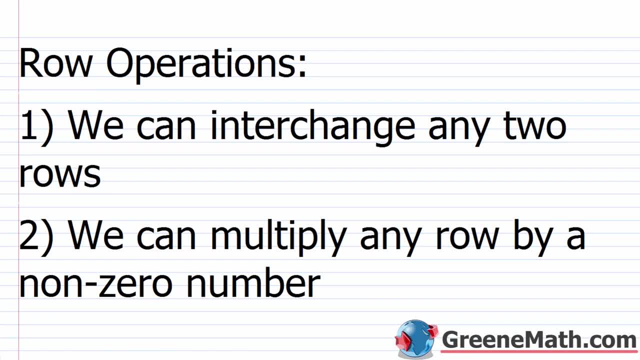 just because it's a little bit cleaner, All right, so let's go down and we're going to talk about the elementary row operations one more time. So the first one is that we can interchange any two rows. That should make sense to you. 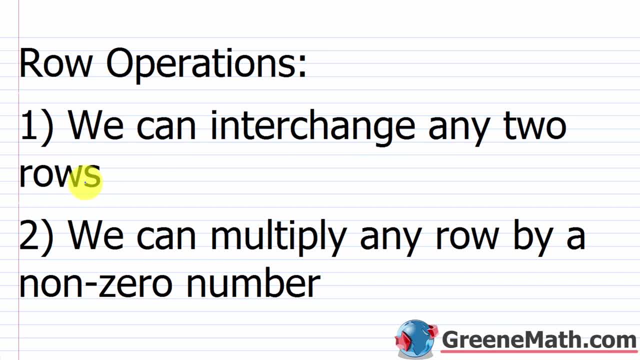 If I'm working with a linear system, it doesn't matter which equation is on top of the other. The second one. we can multiply any row by a non-zero number. This is the same thing as if I multiplied both sides of the equation by a non-zero number. 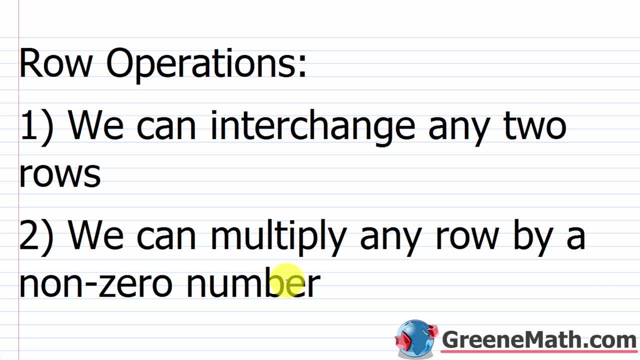 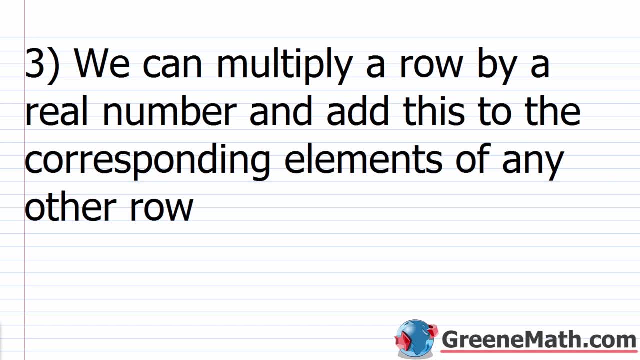 It's the same thing, So we can do that with a row as well. So the last row operation we're going to talk about, row operation three, is a little bit challenging to understand. So we have here that we can multiply a row. 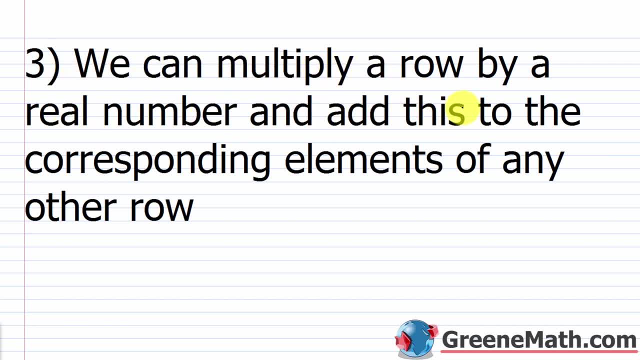 by a real number and add this to the corresponding elements of any other row. So when people first see this, they say: well, what makes this legal? Well, essentially we're using the same basic principles that we use when we use the elimination method. 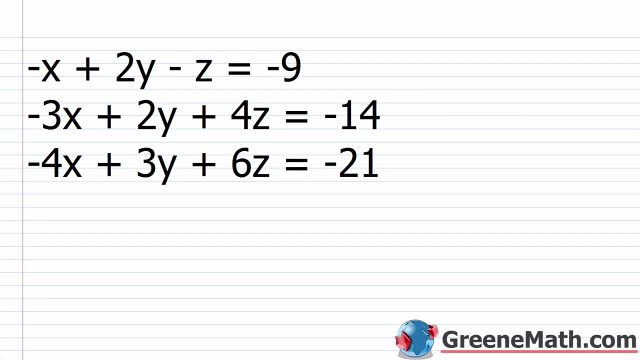 So let's take a look at the first example now So you'll notice how I have everything already written for you in standard form. So you have ax plus b plus by plus cz equals d, where a, b, c and d just represent real numbers. 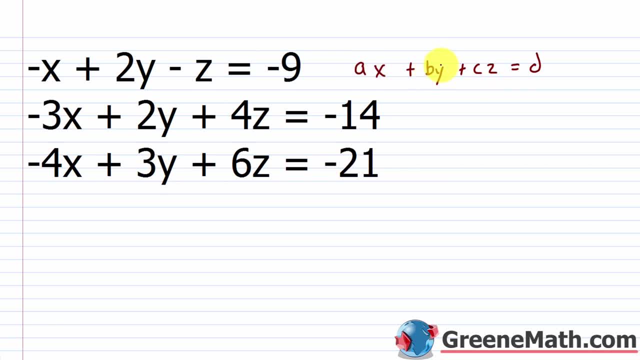 a is the coefficient for x, b is the coefficient for y, c is the coefficient for z, and d is just some constant. Everything is lined up and it's very important that you do that so that you put your information in the matrix correctly. 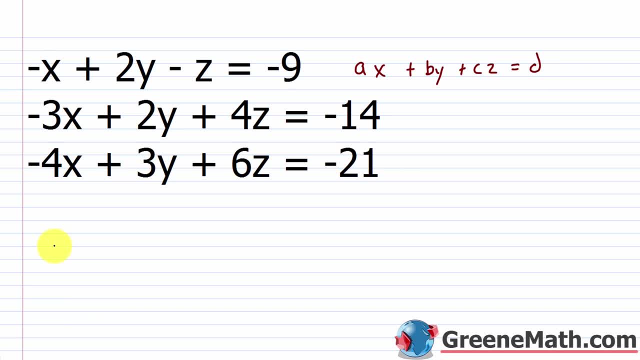 So we're going to write an augmented matrix. So I'm just going to go row by row. So in the first row I have negative 1 as my coefficient for x, So I'll write a negative 1.. Then I have 2 as my coefficient for y. 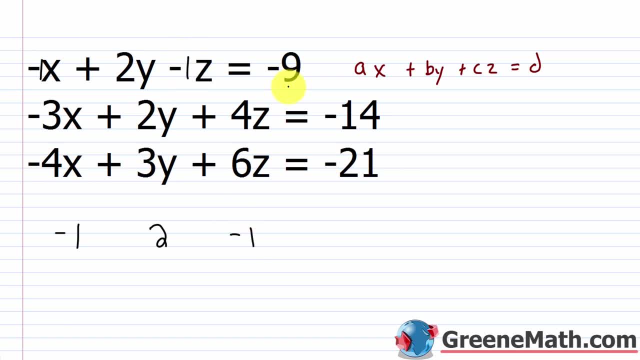 I have a negative 1 as my coefficient for z And then I have a negative 9 as my constant And I just match that. So I have a negative 3.. I have a 2.. I have a 4. And I have a negative 14.. 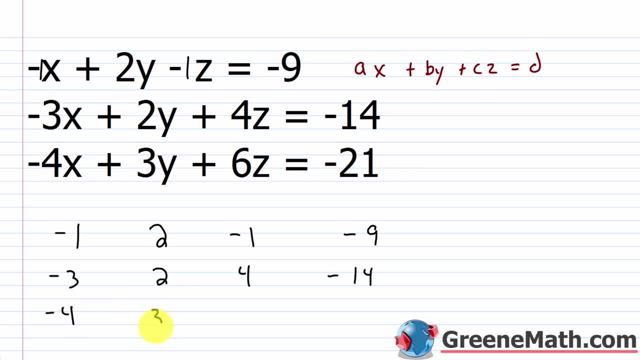 Then I have a negative 4. I have a 3.. I have a 6. And I have a negative 21.. Now, with an augmented matrix, what we want to do is put a vertical bar that separates the coefficients from the constants. 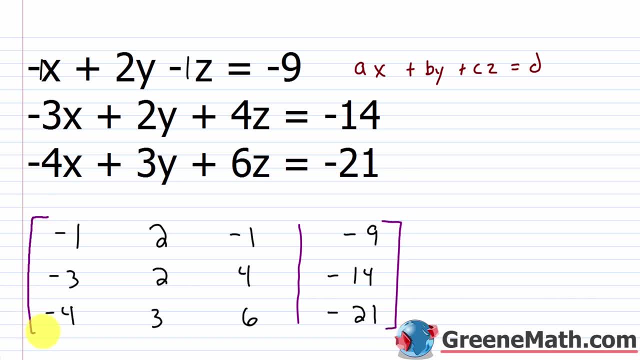 Now I'm going to put my two brackets, one on each side, and I have my augmented matrix. But notice how this works. In this first column, the column all the way to the left, we see that that's all the coefficients for the x variable. 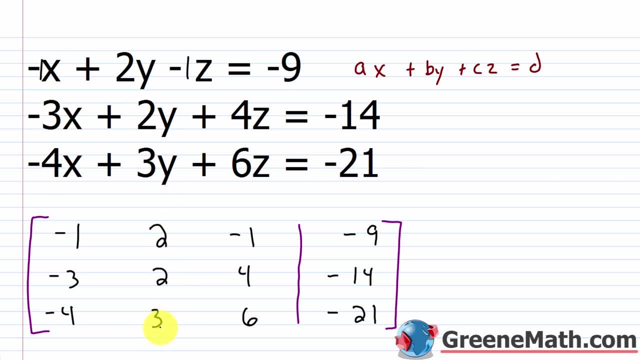 Then, moving 1 to the right, all the coefficients for the y variable, Then all the coefficients for the z variable, Then all the constants. And that's made possible because, again, everything is in standard form, And it's very important that you do that. 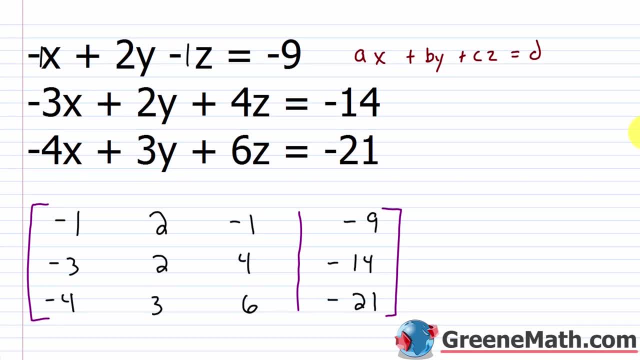 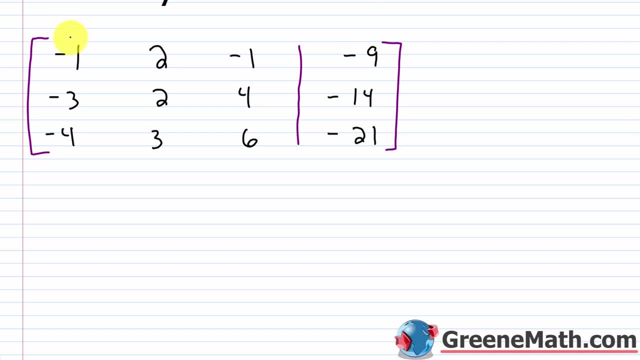 otherwise you're not going to get the right answer. Alright, so once we've done that, what we want to do is work one column at a time. So I start all the way on the left and I concentrate on this first guy right here. 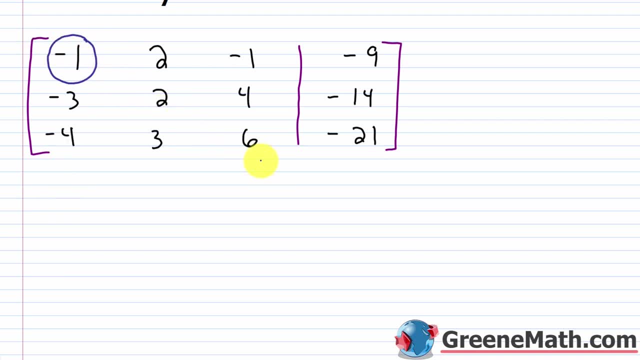 Remember, we want ones going down the diagonal, So I want this to be a 1.. What row operation can I use to produce that? Well, if I multiply negative 1 times negative 1, that would give me 1.. 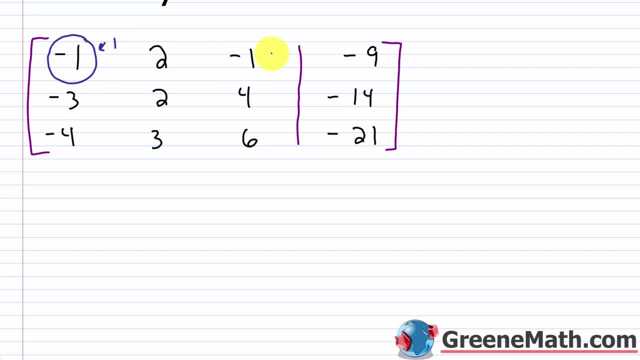 But I can't just multiply this by negative 1.. I've got to do it to the whole row to make it legal. So I'm going to do negative 1 times negative 1, that's 1.. Negative 1 times 2,. 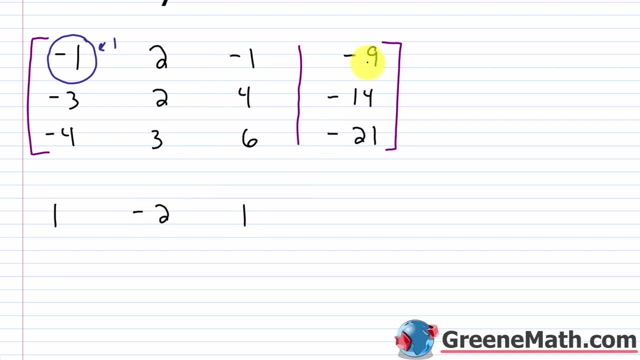 that's negative: 2. Negative 1 times negative: 1 is 1.. Negative 1 times negative: 9 is 9.. Now all the other rows would be the same. So this is negative 3.. This is 2.. This is 4.. 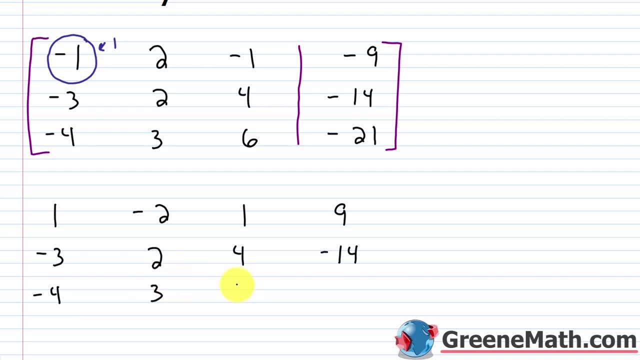 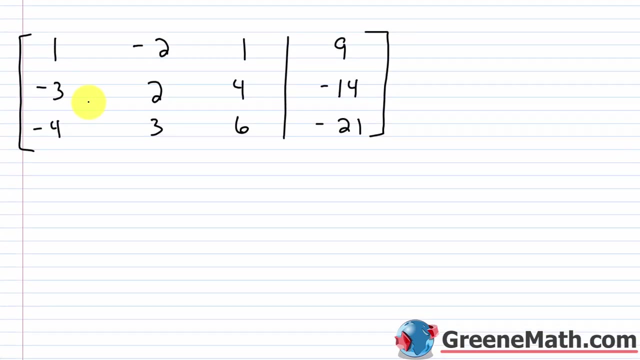 This is negative 14. This is negative 4. This is 3.. This is 6.. This is negative 21.. Alright, Let's scroll down. Get a little room going. So now the next thing: if I'm working a column at a time, 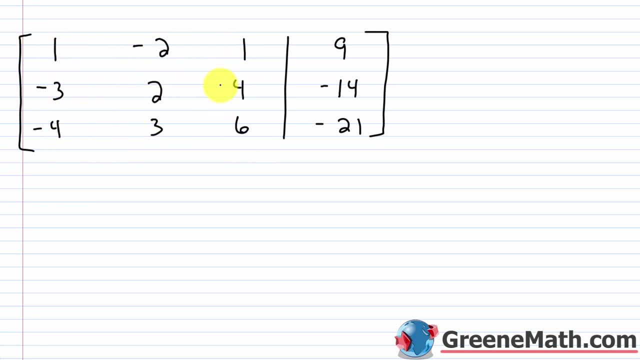 remember one's down the diagonal. I want zeros beneath and above, Depending on what you want to do. I'm going to use the echelon form to make it a little easier for us. So I want zeros beneath and above the diagonal. 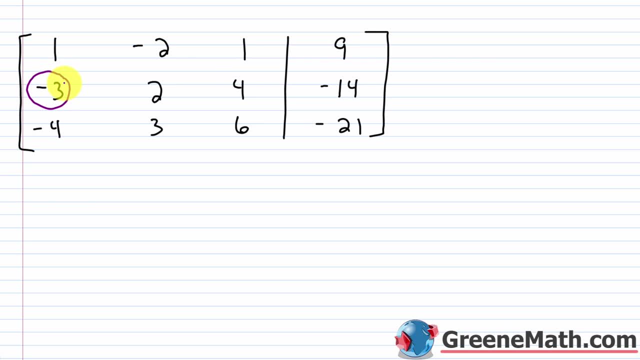 So I want this to be a zero. So what row operation can I use to achieve that? Well, now we're going to think back to our elimination method. Remember if we were trying to eliminate a variable and we didn't have opposite coefficients already on that variable. 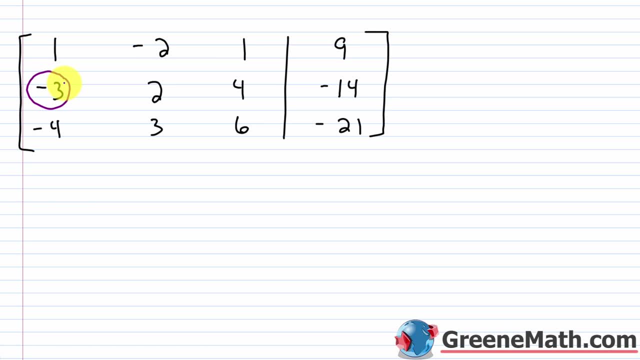 what we had to do is we had to create that, So we would look at transforming one or both of the equations and compare variable terms would cancel. In this case. all I need to do is look at row 1.. If I look at row 1,, 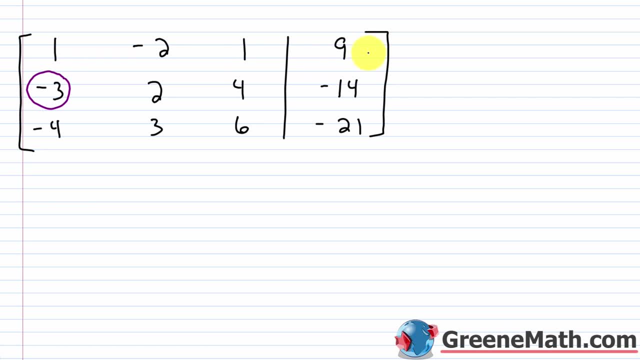 I could multiply row 1 by 3, and then I could add the result to row 2.. Because 3 plus negative 3 would give me 0. So if I multiply 1 by 3, I would get 3.. So that's where that comes from. 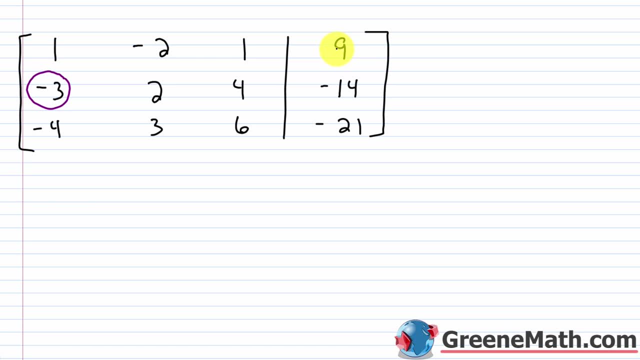 So multiply row 1 by 3.. Now I don't have to actually change row 1.. I just want to keep that the same because the information would be the same. So I already have my 1 here. I don't want to change that. 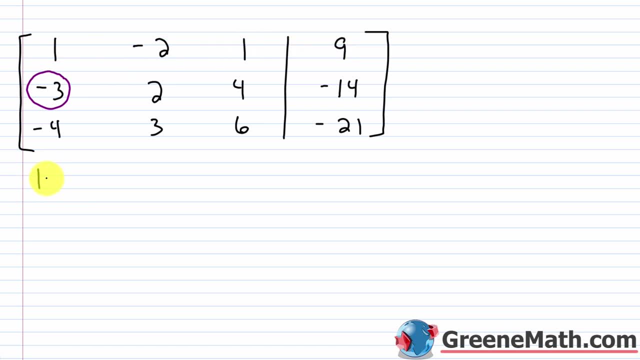 I just want to use the information to make this a 0.. So multiply row 1 by 3.. So I would have 1 times 3,, which gives me 3.. I would have negative 2 times 3,, which gives me negative 6.. 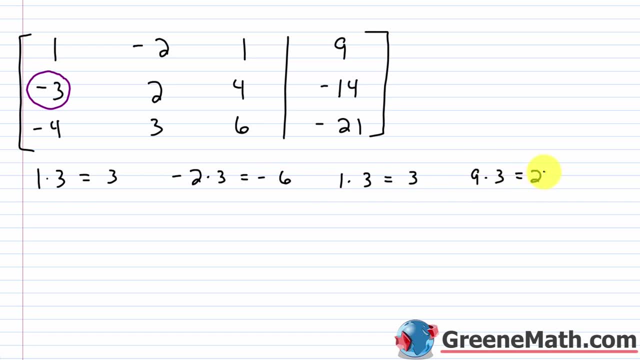 I would have 1 times 3,, which gives me 3.. And I would have 9 times 3,, which gives me 27.. So row 1 itself, again, is going to stay the same. That doesn't change. 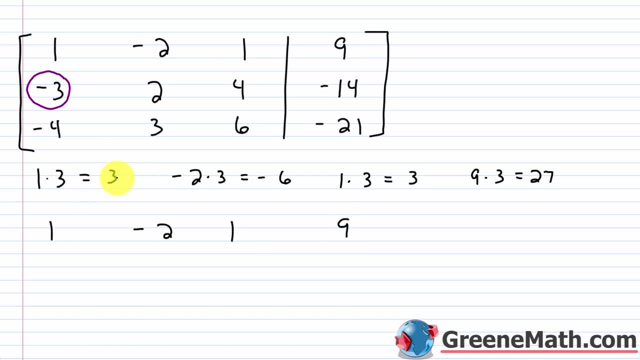 For row 2, I'm adding the result from the multiplication to what's previously there. So negative 3 plus 3 is 0.. 2 plus negative 6 is negative 4.. 4 plus 3 is 7.. Negative 14: 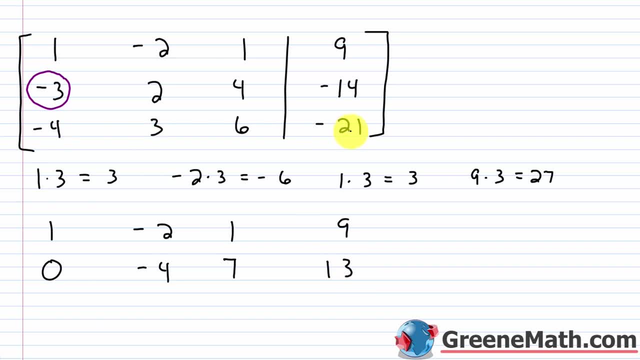 plus 27 is 13.. Now row 3 just remains the same. So we have negative 4,, we have 3,, we have 6, and we have negative 21.. All right Now if I'm continuing in this column. 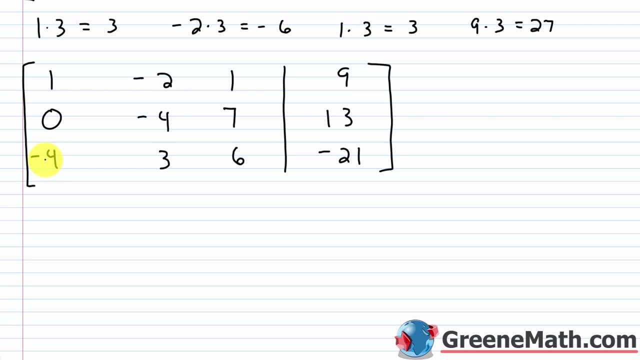 remember, I want this to be a 0 as well, So I'm going to do basically the same thing. So how can I eliminate this? How can I make this a 0?? Well, negative 4 plus 4 is 0.. 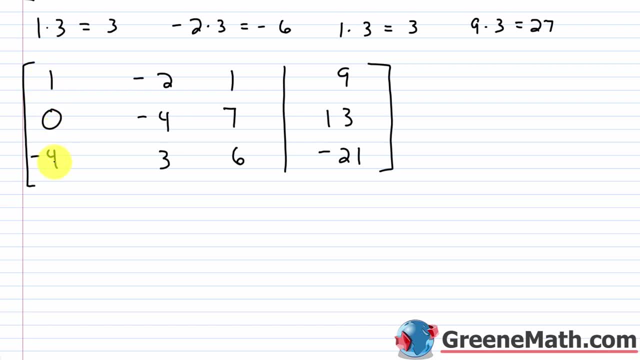 So if I multiply row 1 by 4,, 4 plus negative 4 would give me 0.. So row 1 times 4.. We'd have 1 times 4, which equals 4.. We'd have negative 2 times 4,. 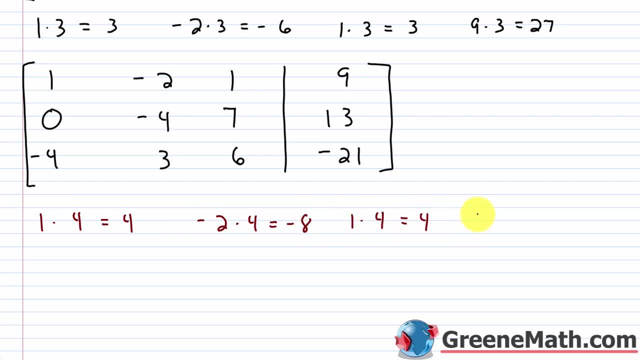 we'd have 1 times 4,, which equals 4.. We'd have 9 times 4,, which equals 36.. So let's go ahead and just replace this row here, And I'll leave these other ones intact. So negative 4 plus 4 would be 0.. 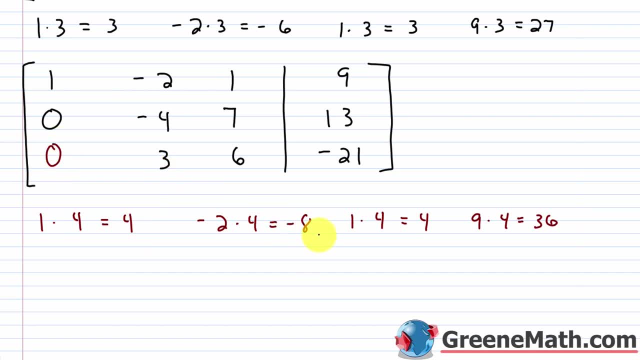 So let's erase this and put 0.. 3 plus negative 8 would be negative 5.. 6 plus 4 would give me 10.. And then negative 21 plus 36 would give me 15.. So this is 15.. 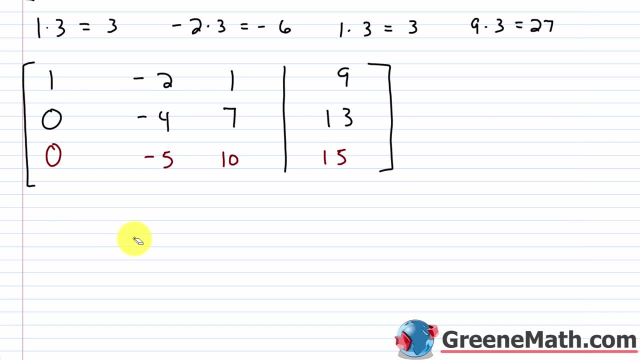 Alright, so let's erase this. Now this column is done, So I want to move one column to the right. Now you might try to start out right here, but typically what I like to do if you get ones down the diagonal. 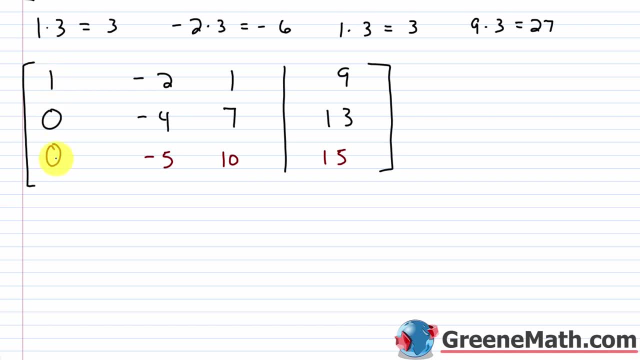 it's easier to work from there. So I started getting a 1 here. then I went down. If I go this way to this column, I want a 1 here. It's very easy to make something into a 1: You just multiply. 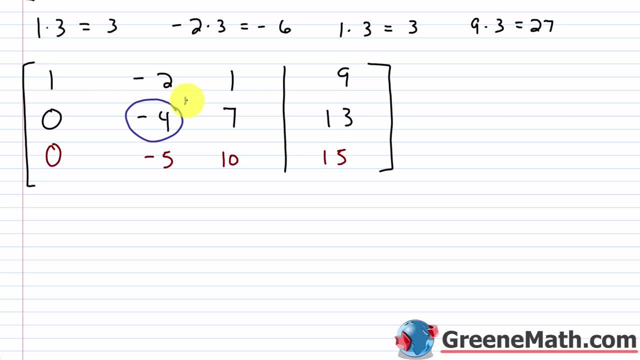 by the reciprocal. So negative 4 times negative 1 fourth would be 1.. And we've got to do it to the whole row. So 0 times negative 1 fourth: 0 times negative 1 fourth is 0. So I can erase that. 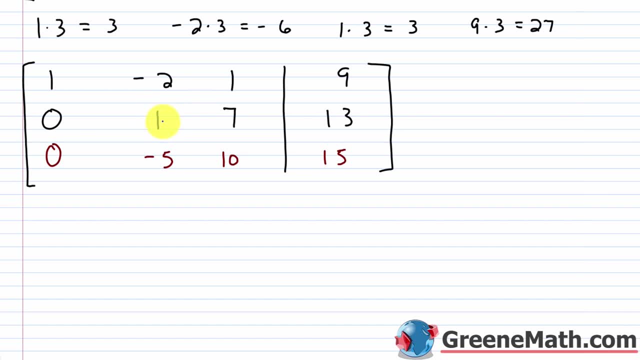 Negative. 4 times negative: 1 fourth is 1.. 7 times negative: 1 fourth is negative 7 fourths. So this is negative 7 fourths, 13 times negative. 1 fourth is negative 7 fourths, 13 fourths. 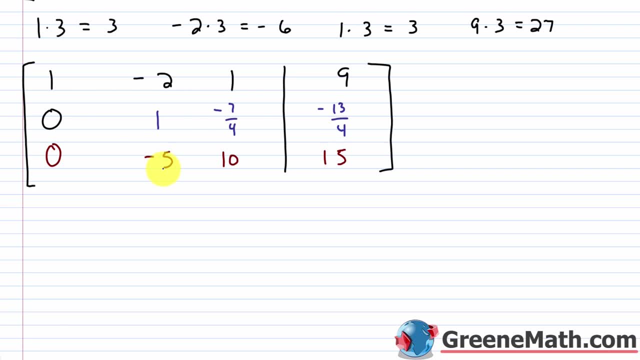 So now that I have a 1 here, I want to get a 0 below and above. So that's pretty easy to do. If I multiply row 2 by 2 and add the result to row 1, I'm going to make this a 0.. 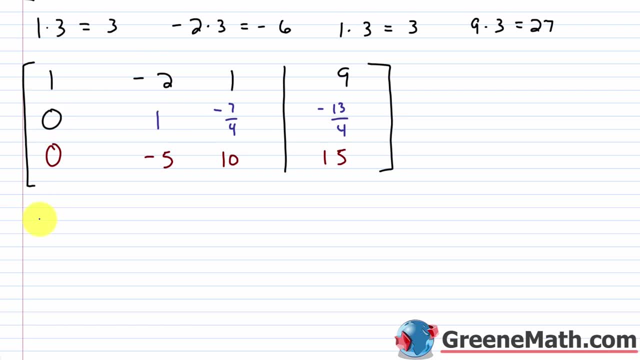 Right. Negative 2 plus 2 is 0. So 0 times 2 would give me 0.. 1 times 2 would give me 2.. Then negative 7 fourths times 2.. 4 cancels with 2. 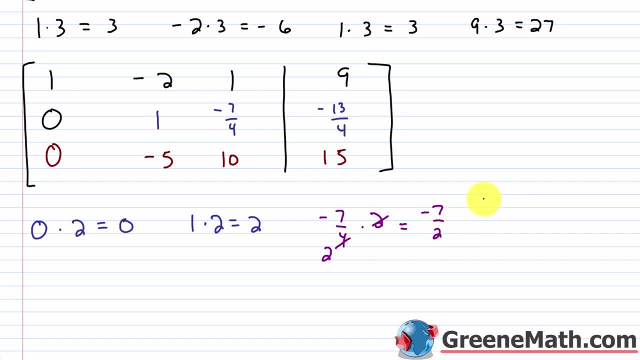 so this equals negative 7 halves And then negative 13 fourths times 2.. Again, this cancels with this and gives me 2.. This is negative 13 halves. So in the first case I'd have 1 plus 0, which is 1.. 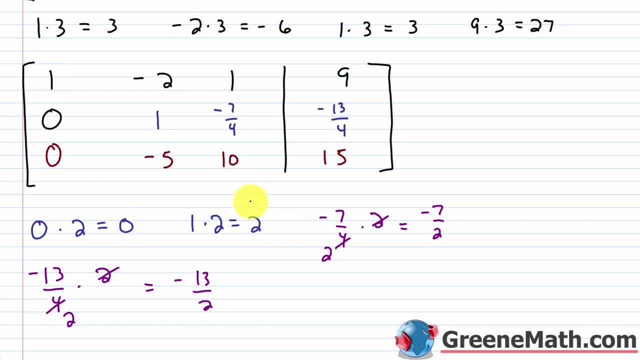 So this stays unchanged, Then I would have 2 plus negative 2, which gives me 0. So this is 0 now. Then I would have negative 7 halves plus 1.. So if I took and erased this and gave myself some room, 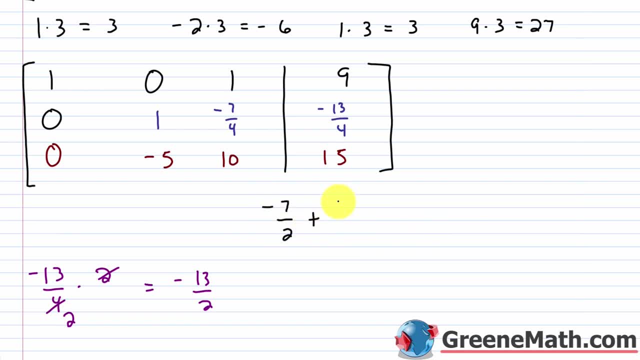 So negative 7 halves plus 1.. I could write 2 over 2 if I wanted to. This would give me negative 5 halves. So this would be negative 5 halves, And then, lastly, we will have 9.. 9 plus negative 13 halves. 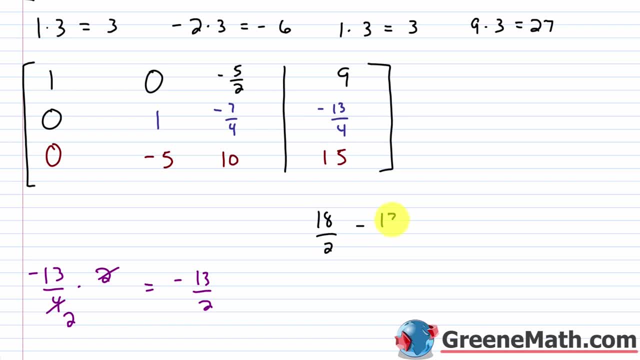 So I'll write 9 as 18 halves minus 13 halves, So this would be equal to 5 halves. So this would be 5 halves. And now let's work on this right here, This negative 5 in this column 2.. 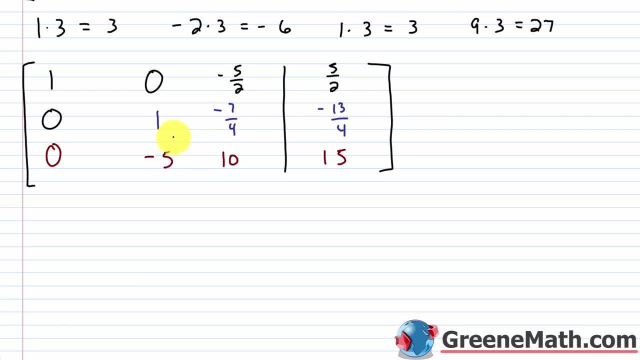 So I can multiply again row 2 by 5. now, 5 plus negative 5 would be 0.. If I do that, when I add the result, I'll get 0.. So 0 times 5 would be 0.. 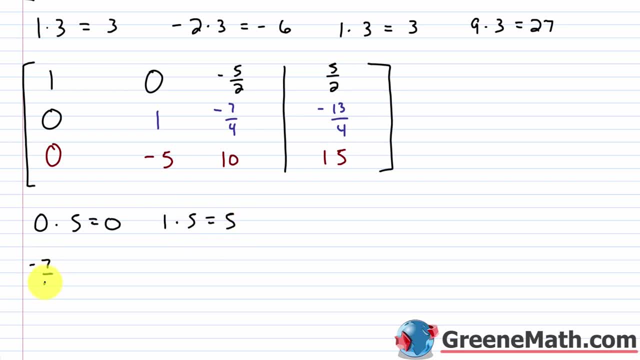 1 times 5 would be 5.. Negative 7 fourths times 5 would be negative 35 fourths. And then negative 13 fourths times 5 would be negative 65 fourths. So we would have 0 plus 0. 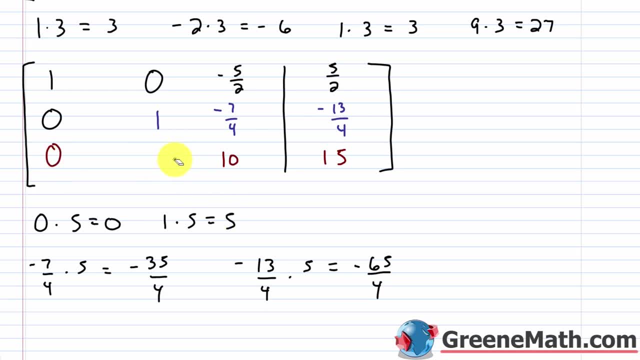 which would give me 0. Then we'd have 5 plus negative 5, which would give me 0. So those two I don't need anymore. Then next I'd have negative 35, fourths plus 10. So negative 35. 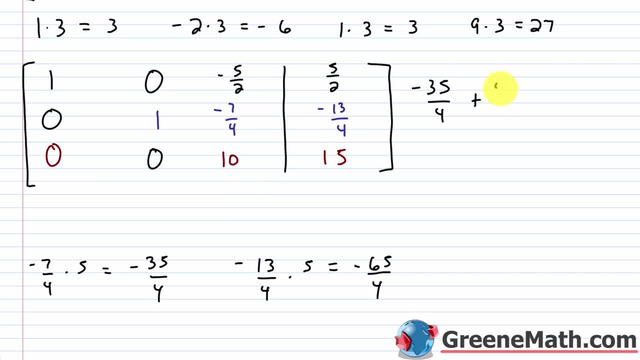 fourths plus for 10, I'm going to write 40 over 4.. So negative 35 plus 40 would be 5.. So you'd have 5 fourths here, So 5 fourths. And then, lastly, let me erase all this- 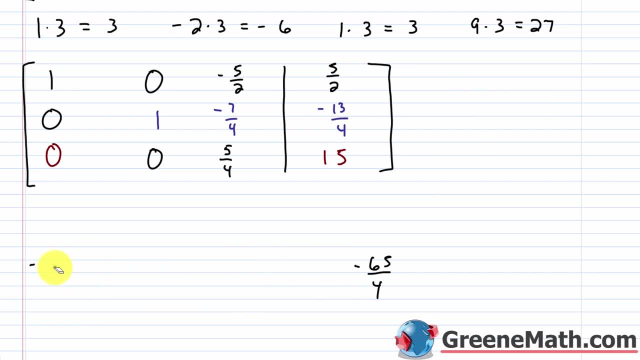 Get some room going, You'd have negative 65 fourths plus 15.. So negative 65 fourths plus For 15. I'm going to write that as 60 over 4.. Negative 65 plus 60 is negative 5. So this would be negative 5. 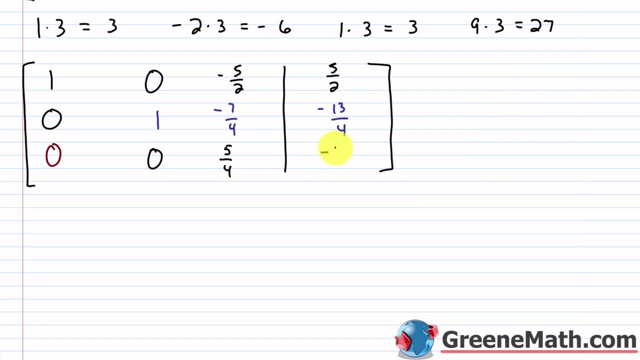 fourths. So it would be negative 5 fourths. Alright, So let's continue. So this column's done, This column's done. So I want to get a 1 right here. Again, it's easiest if you just do the diagonals. 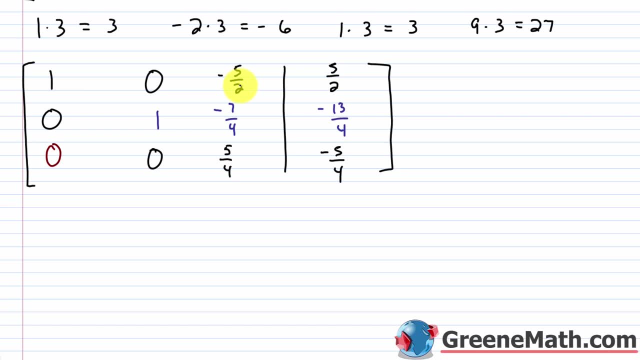 with a 1 first and then make your zeros, So for 5 fourths. how do I get that into a 1?? Well, I multiply by the reciprocal, So that's 4 fifths. 0 times 4 fifths is. 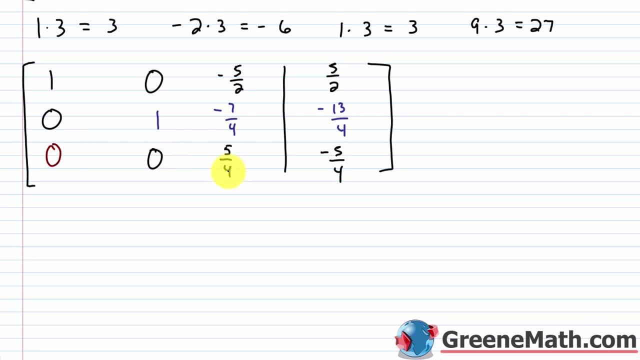 0. 0 times 4 fifths is 0.. 5 fourths times 4 fifths is 1.. Negative: 5 fourths times 4 fifths is negative: 1.. So, although we know at this point that z equals negative, 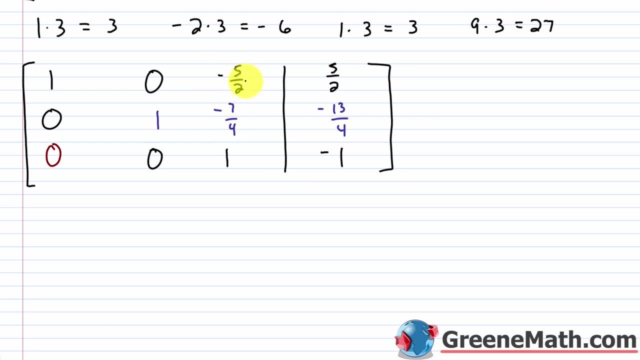 1, we want to continue and get zeros here and here so that we don't need to go back and use substitution. So how do I go about getting a 0 here? Well, if I multiply 1 by 7 fourths, I can add 7 fourths to negative 7. 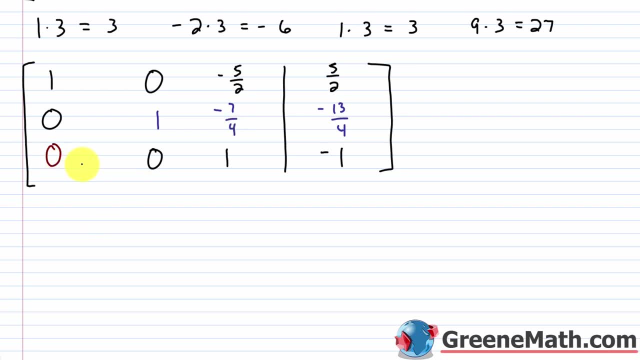 fourths and I would have a 0 there. So if I multiply row 3 by 7 fourths, 0 times 7 fourths equals 0.. Then 0 times 7 fourths equals 0.. Then 1 times 7 fourths equals. 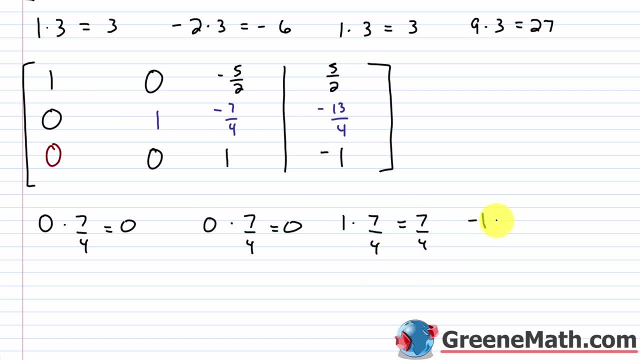 7 fourths And then negative 1 times 7 fourths equals negative 7 fourths, So I'm going to add the results to row 2.. So 0 plus 0 is 0.. Get rid of that. 0 plus 1 is 1.. 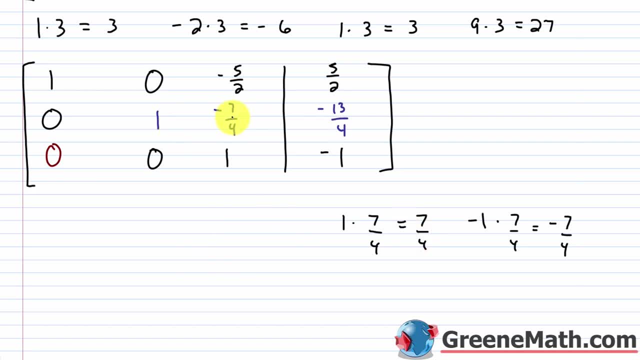 Get rid of that. 7 fourths plus negative 7 fourths is 0. So that's gone. And then I'd have negative 7 fourths. so negative 7 fourths plus negative 13 fourths. Negative 7 plus negative 13. 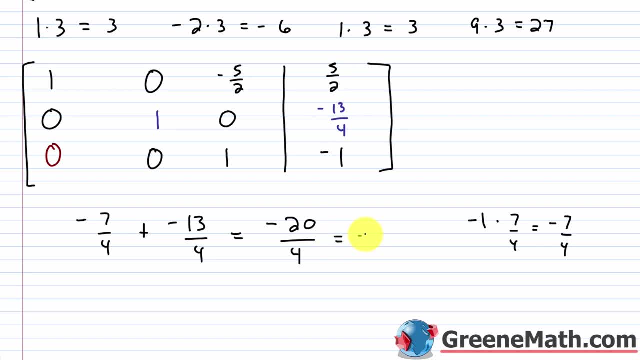 would be negative 20. This is over 4, so this equals negative 5.. So this right here is negative 5.. So now we know that y, ok y, because x and z the coefficients are 0, so this would be 1y or just y. 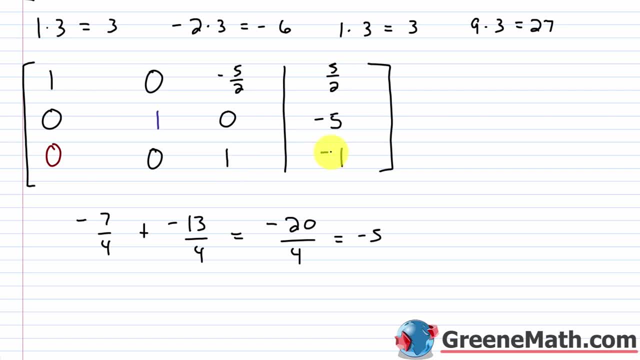 would be equal to negative 5.. So I know z is negative 1, y is negative 5.. Now we just need to figure out what x is. So let's erase all this. So my last step here is just to figure out. 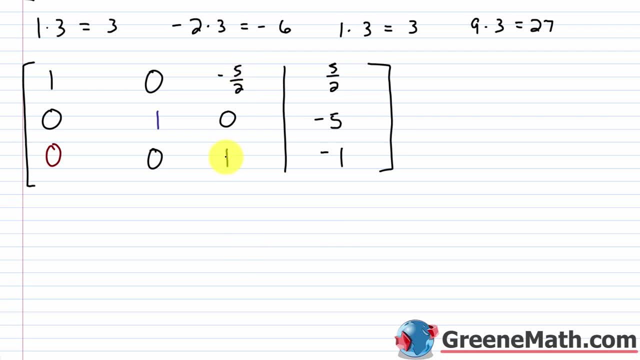 how to get a 0 right here, And all I need to do is multiply 1 by 5 halves and add that result to negative 5 halves and I would have a 0 right there, and I'm done. So I'm going to multiply. 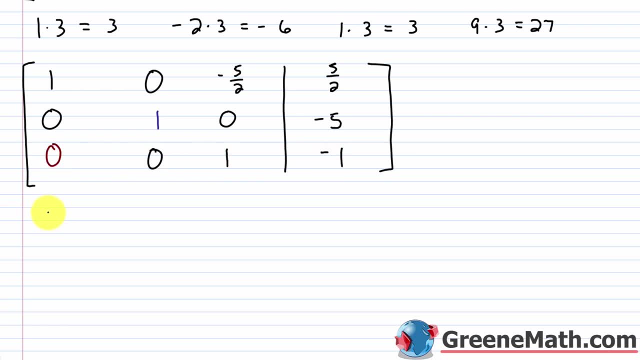 row 3 by 5 halves. 0 times 5 halves is 0.. 0 times 5 halves is 0.. 1 times 5 halves is 5 halves. 5 halves plus negative 5 halves is 0.. 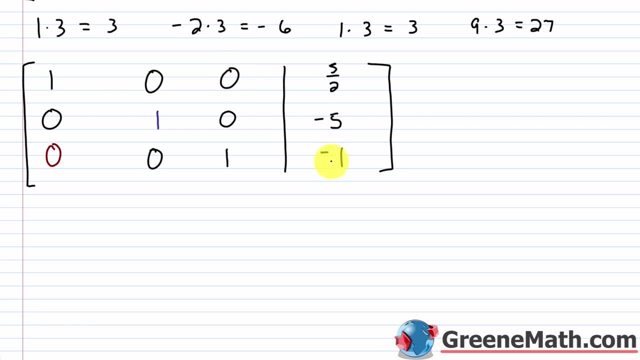 So this would be 0.. Negative 1 times 5 halves is negative 5 halves. So this would give me negative 5 halves, and I would add that to 5 halves here, That would give me 0 as well. So what we have now? 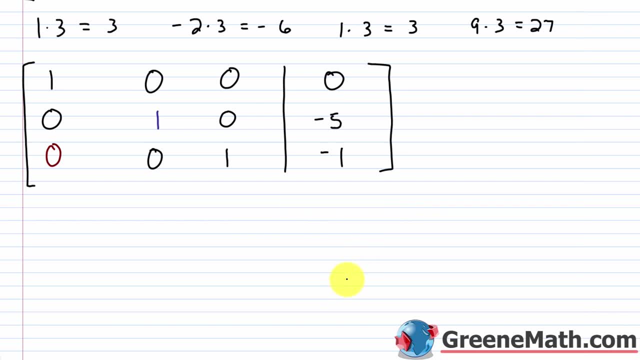 is reduced row echelon form. I have 1s down the diagonal, I have 0s below and 0s above, And why this is convenient. if I think about this again, the information is written as ax plus by plus. cz equals d. 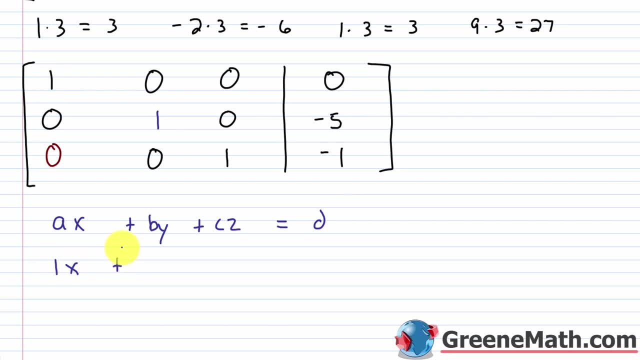 So I know this is the coefficient for x. So 1x plus this is the coefficient for y: 0y plus this is the coefficient for z: 0z equals. then I have a 0.. So essentially, these are gone and I basically have 1x or just x equals 0. 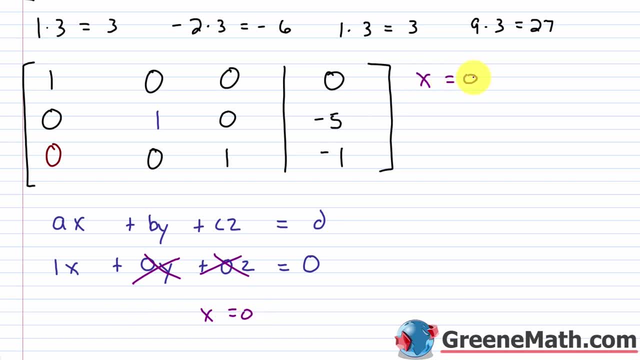 So x equals 0.. Then I know that y, which again this coefficient in the middle is the coefficient for y- is equal to negative 5 and z is equal to what? This is the coefficient for z. So 1z equals negative 1.. So z equals negative 1.. 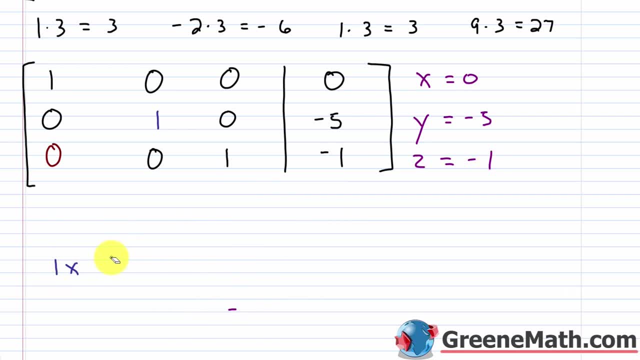 So, as an order triple, if you want to write it that way, your solution here is: 0 comma negative, 5 comma negative, 1.. It's x, y, z. Alright, so let me check this first result. I'm not going to check any of the 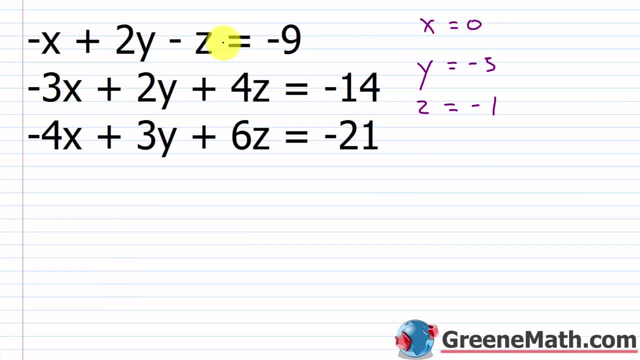 ones after this, but I do want to check this one. Alright, so for the first equation I'm going to plug in a 0 for x, So I'd have negative 0, which is just 0. So don't even worry about that. Then I'd have 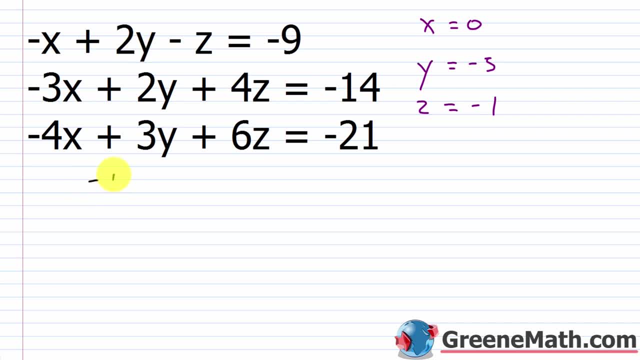 2y. So y is negative 5.. 2 times negative 5 is negative. 10 minus z, z is negative 1.. So minus the negative 1 is plus 1.. This should equal negative 9, and it does. So it checks out here. 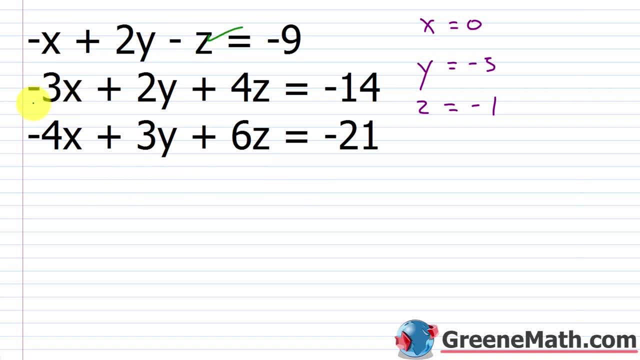 In the second equation, negative 3 times 0 is 0. So this would be gone. You'd have 2y. y is negative 5, so that'd be negative. 10 plus 4z, z is negative 1. So 4 times negative, 1 is negative. 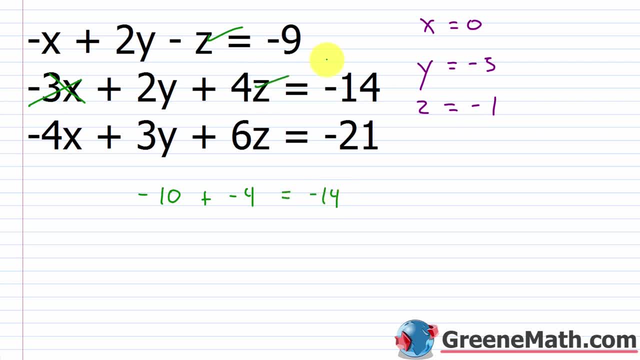 4. So this equals negative 14, and it does For the final equation. we have negative 4x. Again, negative 4 times 0 would be 0. So this would be gone. You'd have 3y 3 times negative. 5 is negative 15, so this would be. 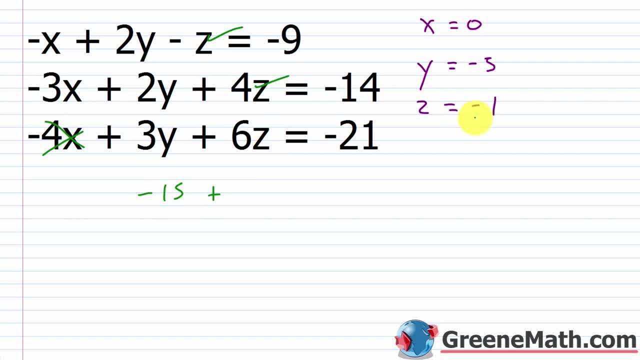 negative 15 plus 6z z is negative 1. So 6 times negative 1 is negative 6. So negative 15 plus negative 6 equals negative 21.. Yes, that's true. So it checks out in every equation. So we verify that this is the. 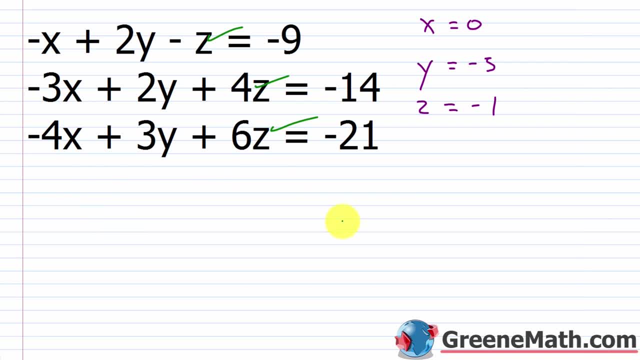 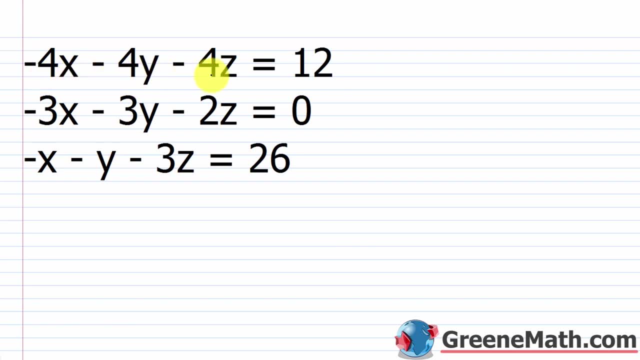 solution for the system: x equals 0, y equals negative, 5, z equals negative, 1.. All right, let's take a look at the next one. So we have negative. 4x minus 4y minus 4z equals 12. We have 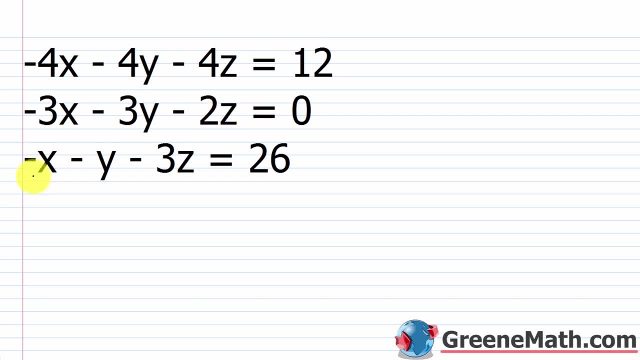 negative 3x minus 3y minus 2z equals 0.. We have negative x minus y minus 3z equals 26.. I have everything written in standard form. It's ax plus by plus cz equals d, So let's write our. 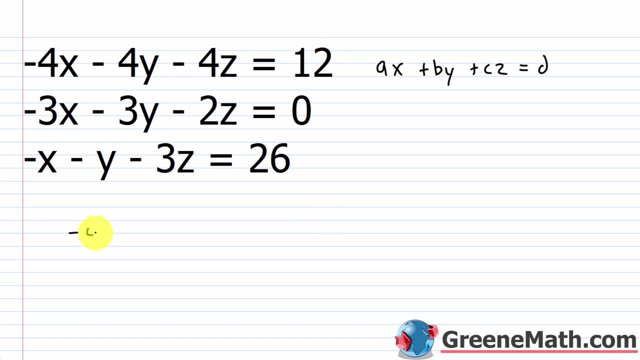 information into the augmented matrix. We'd have negative 4, we'd have negative 4, we'd have negative 4, and we'd have 12. We'd have negative 3, negative 3, negative 2, and then 0. We'd have 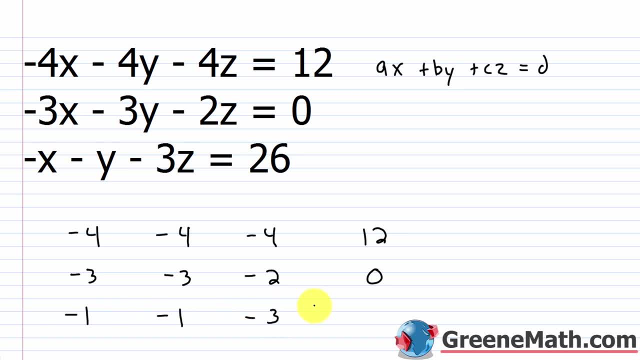 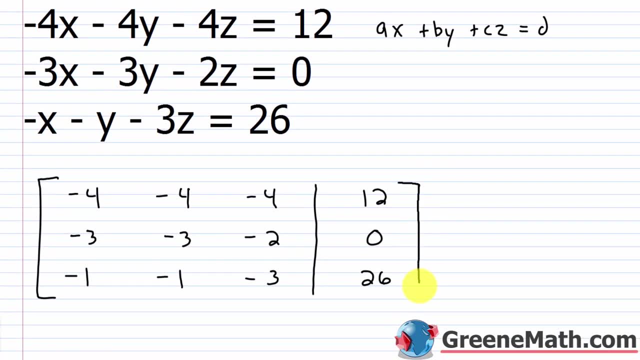 negative 1,, negative 1,, negative 3, and you'd have 26.. All right, Remember. this vertical bar here just separates the coefficients from the constants. So we've set up our augmented matrix. So what do we do now? Remember? 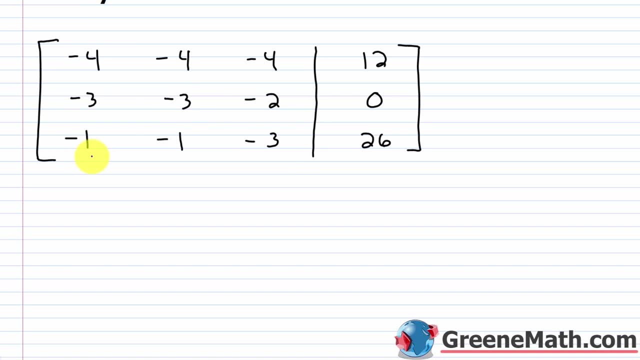 we want 1s down the diagonal. We want 0s below and above. So how do I get negative 4 changed into a 1?? Well, I multiply by the reciprocal. The reciprocal of negative 4 is negative 1 fourth. So if I just multiply by the reciprocal of negative 4, I get negative 1 fourth. 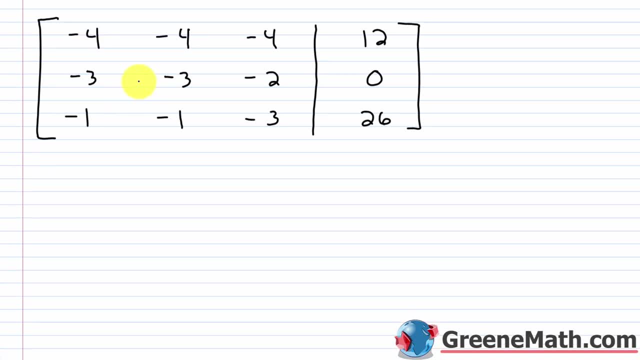 So I can just erase all of these and just put 1s, And then this would be what: 12 times negative 1. fourth would be negative 3.. Next, I want to make this into a 0. So if I want this to be a 0,, 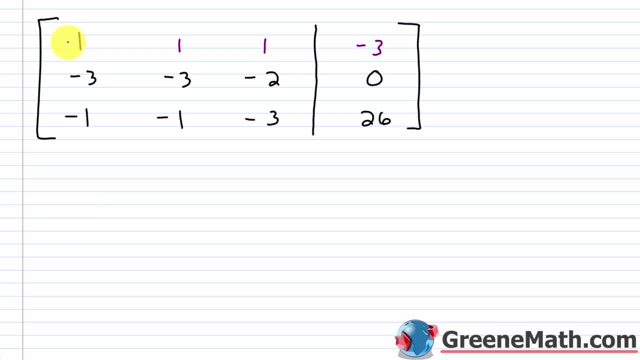 what can I do? Well, I can multiply row 1 by 3.. Because if this was multiplied by 3, I'd get 3,. 3 plus negative 3 would be 0.. So if I multiply row 1 by 3, I'd have 1 times 3, which equals 3,. 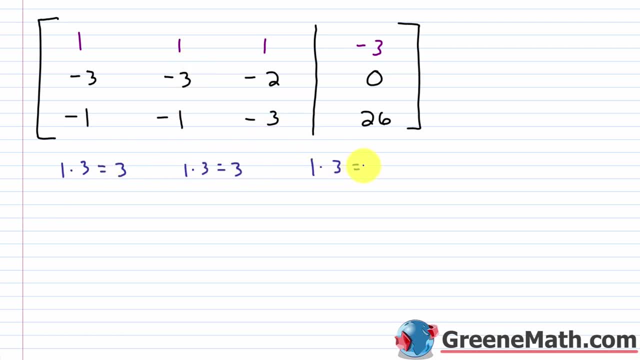 1 times 3,, which equals 3,, 1 times 3,, which equals 3, and negative 3 times 3,, which equals negative 9.. So I add the results: 3 plus negative 3 is 0.. 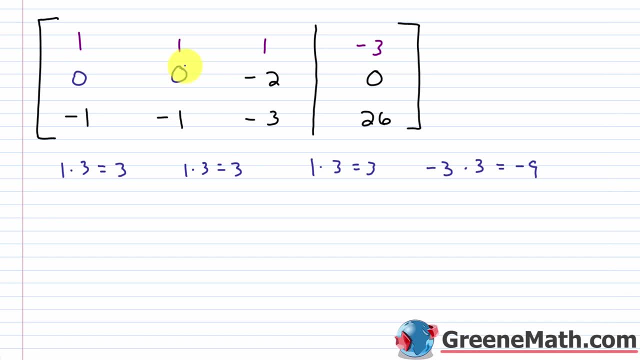 Then negative 3 plus 3 is 0.. Then 3 plus negative 2 is 1.. Then negative 9 plus 0 is 0.. All right, so what would I do next? Well, now I want to make this into a 0.. So I can multiply row. 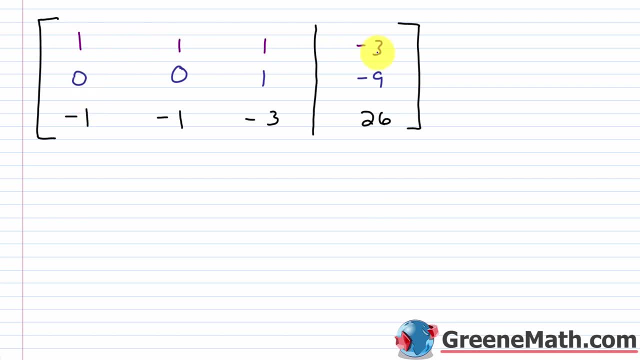 1 by positive 1 and add it to row 3.. So 1 times 1 is 1.. 1 times 1 is 1.. 1 times 1 is 1.. And negative 3 times 1 is negative 3.. So 1 plus negative 1 is 0.. Negative 1 plus 1 is 0.. 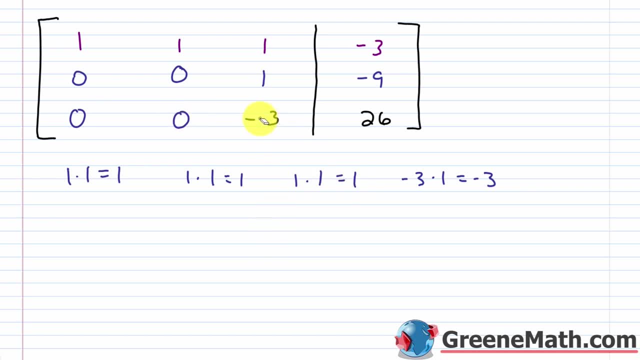 Negative 3 plus 1 is negative 2.. And negative 3 plus 26 is 23.. Now, before we go any further and waste any more time on this problem, I want to point out the fact that this right here is a 0. That should signal to you that. 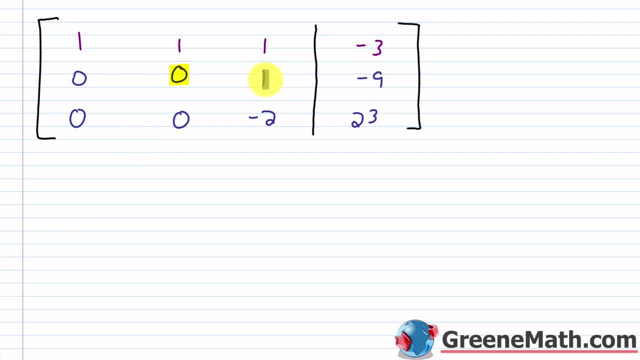 you have a problem already. Right now you have 1z equals negative 9.. So z equals negative 9. According to row 2.. If I look at row 3, I have negative 2z equals 23.. If I plugged in a negative 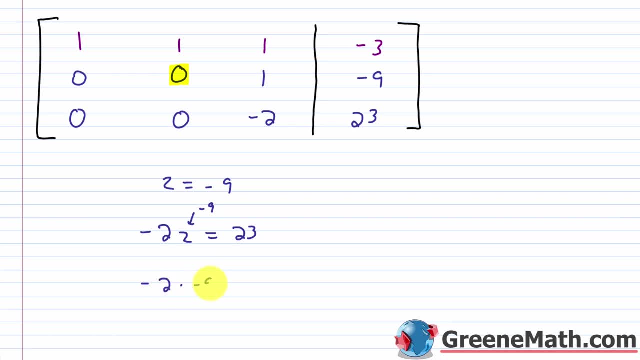 9 here. what would I get? I'd get negative 2 times negative: 9 equals 23.. I would get 18 equals 23, which is false. Okay, I end up with a nonsensical statement. So this is an inconsistent system. 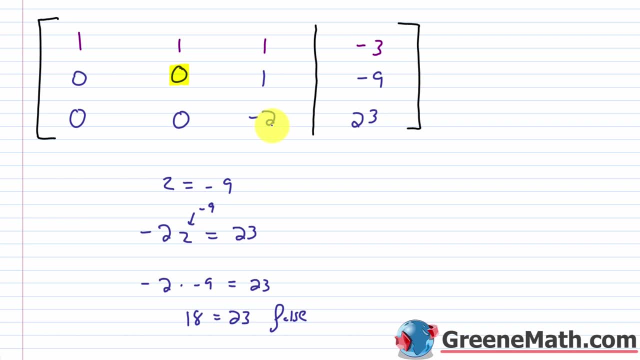 When you start to get information that doesn't make sense, just stop. Okay, stop, Do what I just did there. You can see, obviously this isn't going to work. You don't need to go any further Now, if you wanted to really prove this to yourself. 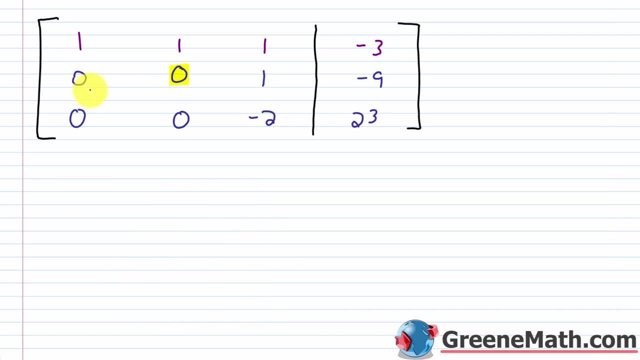 you could multiply row 2 by 2, and you could add to row 3.. 0 times 2 is 0.. 0 plus 0 is 0. So this would stay the same. 0 times 2 is 0.. 0 plus 0 is 0.. So this would stay the same. 1 times 2 is 2.. 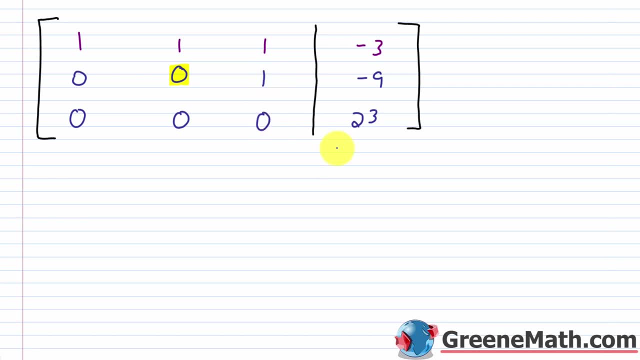 2 plus negative 2 is 0. So this would be a 0. And then if 9 times 2 is negative 18, negative 18 plus 23 would give me 5.. So what does this tell me here? 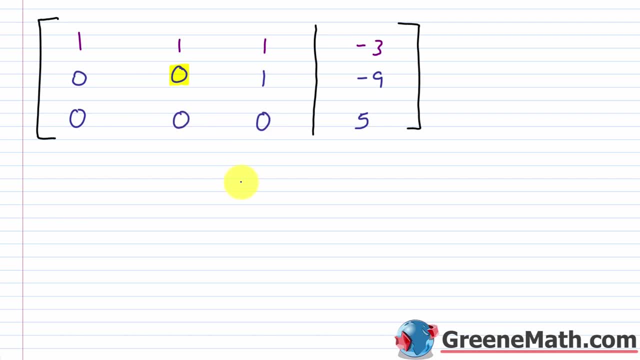 0x plus 0y plus 0z. So basically 0 is equal to the constant 5. That's false. Okay, again you start seeing stuff like this. You can stop and say: does this make any sense? 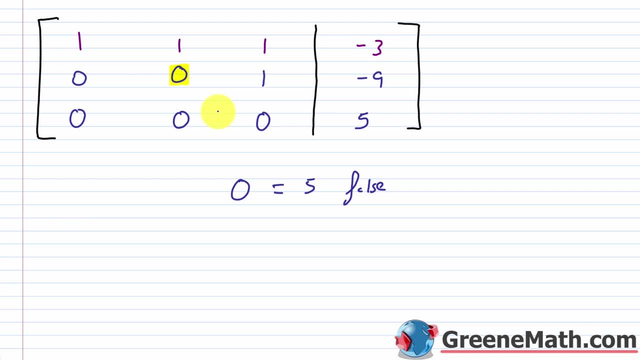 Plug in what you know so far and you can obviously see that you get a nonsensical statement. And so there is no solution. There is no solution. All right, let's take a look at one more. So we have x minus 3y plus 6z equals 11.. 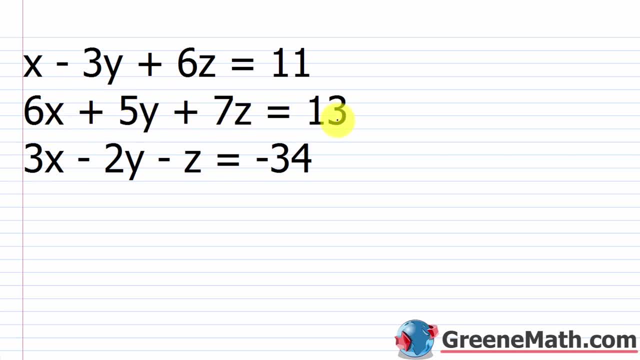 We have 6x plus 5y plus 7z equals 13.. We have 3x minus 2y minus z equals negative 34.. So what you want to do again, everything is already in standard form. Just put the information into the augmented matrix, So we'll have a 1,. 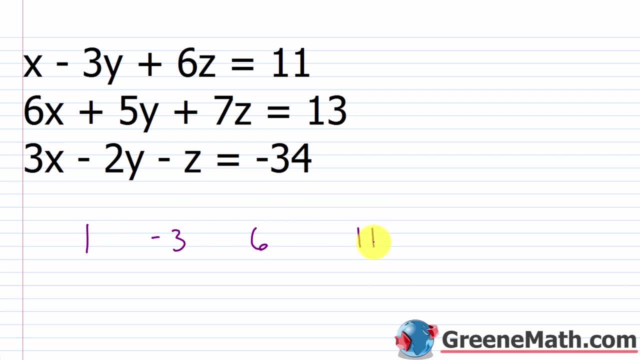 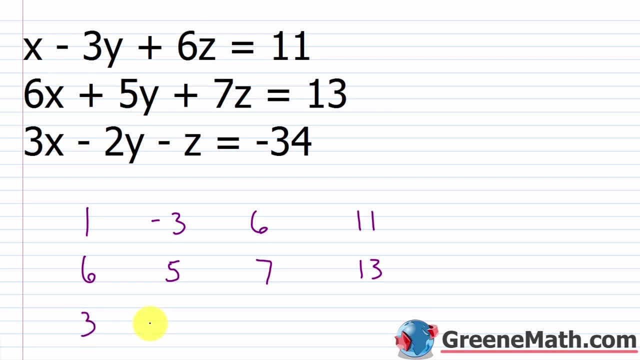 a negative 3,, a 6, and an 11.. We'll have a 6,, a 5,, a 7, and a 13.. We'll have a 3, a negative 2,, a negative 1, and a negative 34.. Put a vertical bar here. 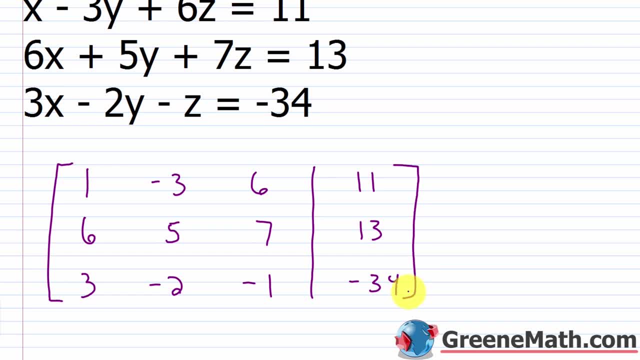 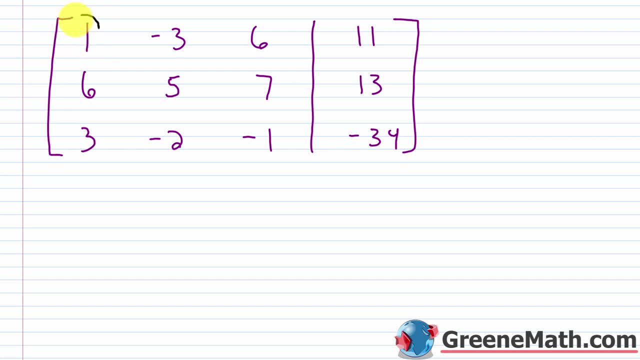 and then brackets on this side and on this side, All right, so let's scroll down a little bit. Now again, I want to start out in this first column here, and this is already a 1.. So I don't remember. I want 1s down the diagonal. That's already a 1, so I move to the 6.. 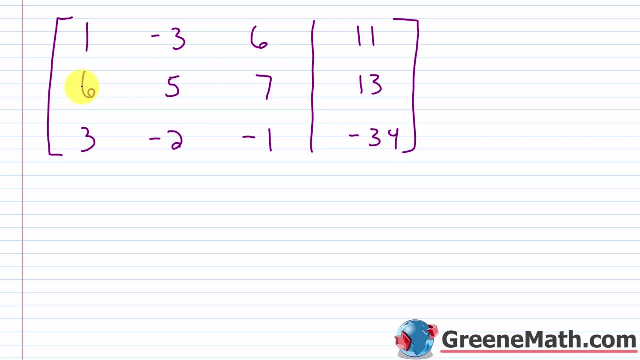 How can I make that 6 into a 0?? Well, 6 plus negative 6 would be 0, and I can multiply this 1 right here by negative 6 to get negative 6.. So if I multiply row 1 by, 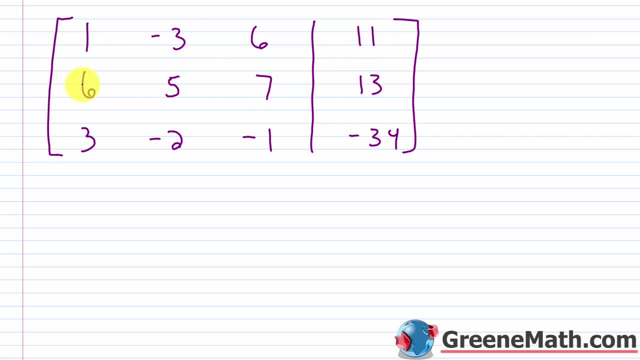 negative 6 and add the result to row 2, I'll have a 0 here. So I'll have 1 times negative 6.. That equals negative 6.. I'll have negative 3 times negative 6,, which would be 18.. I'll have 6 times. 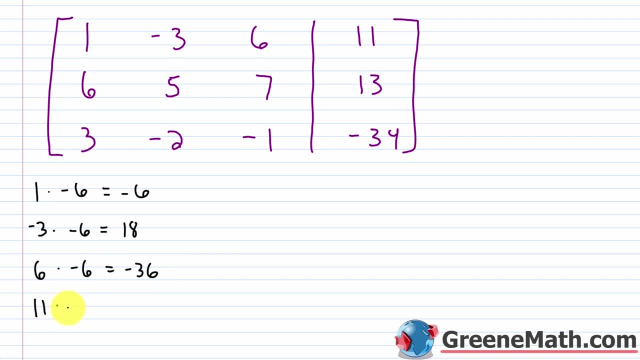 negative 6,, which would be negative 36.. And I'll have 11 times negative 6,, which would be negative 66. So I'm going to add: 6 plus negative 6 is 0. So this is 0.. 5 plus 18 is 23.. Negative: 36 plus 7. 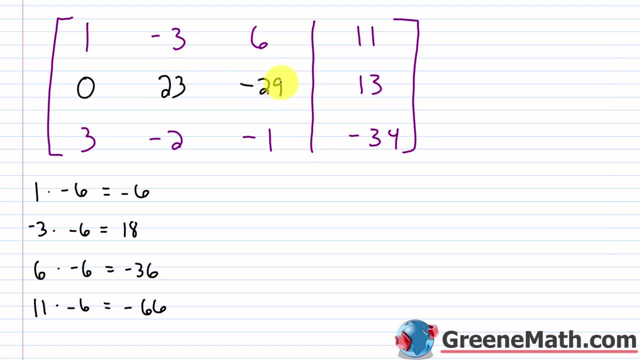 is negative 29.. And then negative 66 plus 13 is negative 53.. All right, so let's erase this. So we continue working in this column. So how can I get this 3 to be a 0?? Well, I can multiply 1. 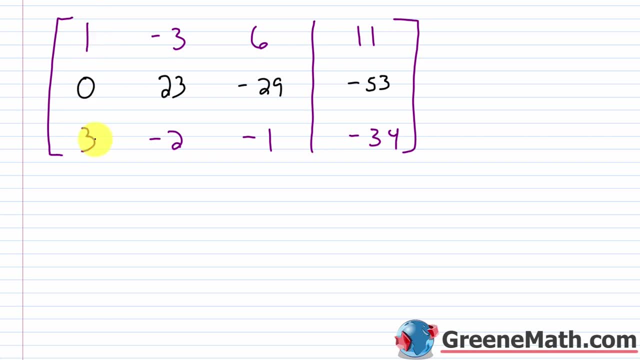 times negative 3.. That would give me negative 3.. Negative 3 plus 3 would be 0.. So if I multiply row 1 by negative 3, it would look like this: 1 times negative, 3 is negative 3.. Negative 3 times negative. 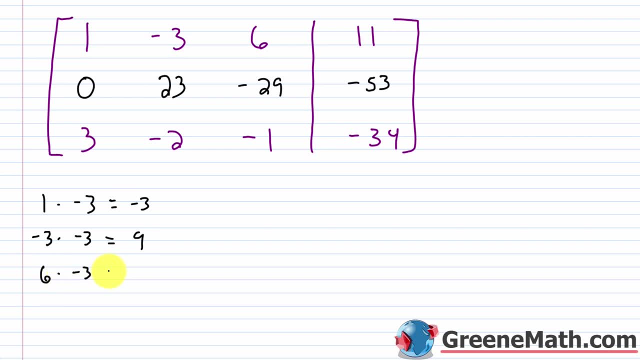 3 is 9.. 6 times negative 3 is negative 18.. And 11 times negative 3 is negative 33.. So we add the results to row 3.. 3 plus negative 3 is 0.. 9 plus negative 2 is going to be 7.. 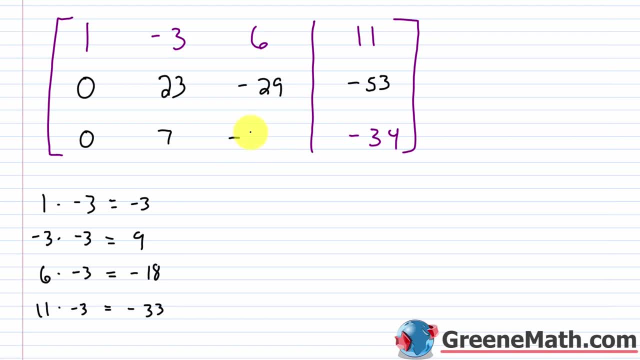 Negative 18 plus negative 1 is negative 19.. And then negative 34 plus negative 33 is going to be negative 67.. This is negative 67 here. Let me erase this. All right. so the first column is done. 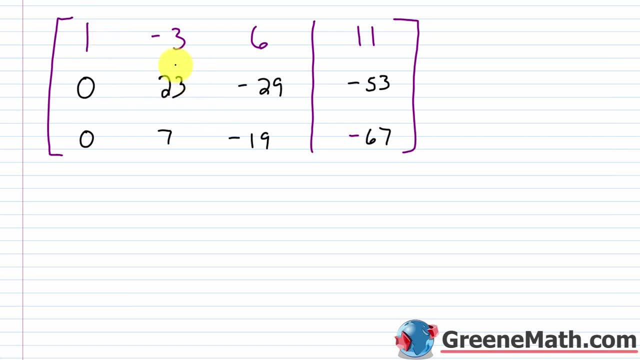 Now I want to go to the second column And again I always want to get a first, So 1's down the diagonal. That just makes things easier. So I can multiply row 2 by 1 over 23.. We'll do a reciprocal of 23 to make this a 1.. 0 times 1 over 23 is 0.. 23 times 1 over 23 is 1.. 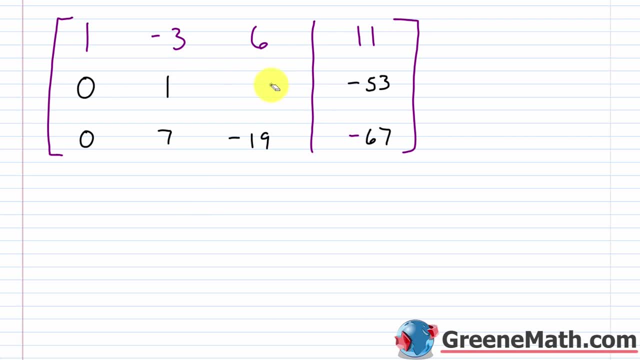 Negative 29 times 1 over 23 would just be negative 29 over 23.. Negative 53 times 1 over 23 would just be negative 53 over 23.. Okay, so now I want a 0 above and below, So it doesn't matter what you. 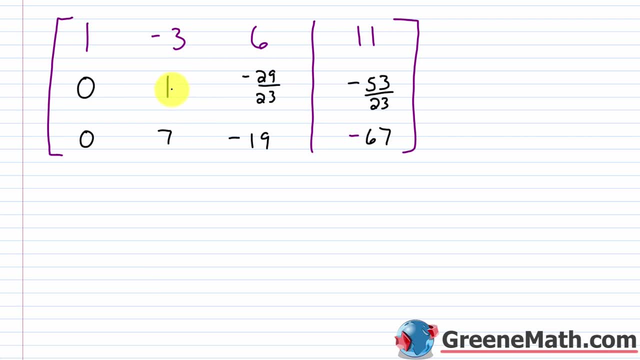 start with, Let's go ahead and just do the one above first. So I would multiply 1 times 3 to get 3 and add 3 to negative 3 to get a 0. So I'm going to multiply row 2 by 3, add the result to. 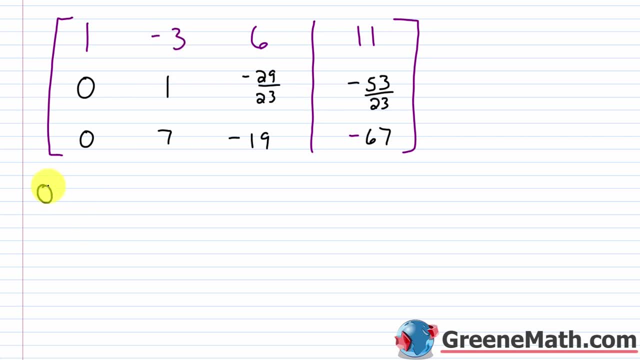 row 1.. So row 2 multiplied by 3.. 0 times 3 equals 0.. 1 times 3 equals 3.. Negative 29 over 23 times 3 is equal to negative 87 over 23.. And then negative 53 over 23 times 3 is going to be equal. 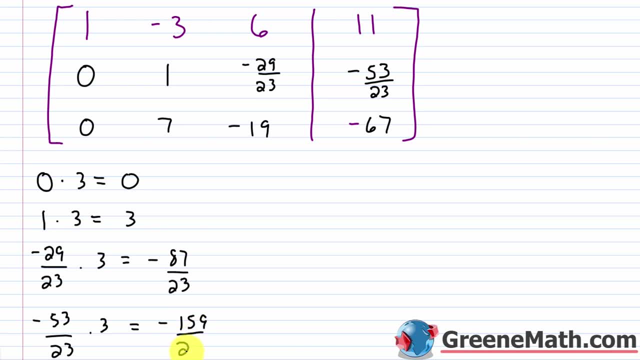 to negative: 159 over 23.. All right, so we're going to add these results: 2 row 1.. So 0 plus 1 is 1.. So I don't need this anymore. I can erase this. 3 plus negative 3 is 0.. I can erase this. Negative 87 over 23 plus 6.. So negative 87 over 23 plus. 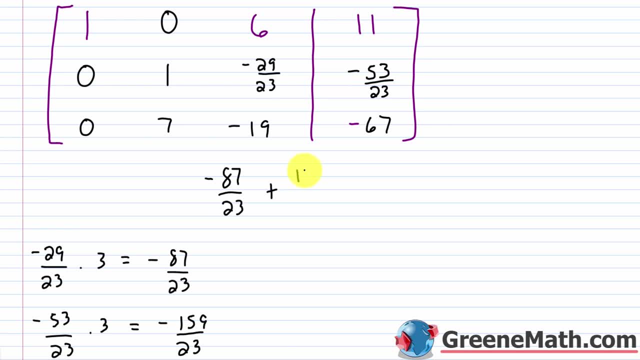 what's 6 times 23?? Well, that gave me 138.. So 138 over 23.. And if I did negative 87 plus 138, that would give me 51. So this is 51 over 23. So 51 over 23.. Let's erase this Now. lastly, we want to do 11 plus. 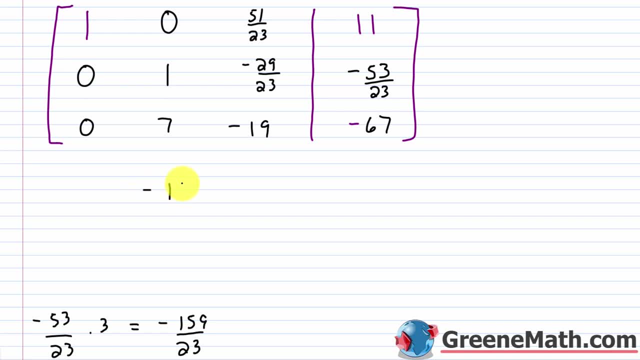 negative 159 over 23.. So negative 159 over 23 plus 11 times 23 is 253.. So 253 over 23.. So 253 minus 159 is 94.. So 253 over 23 is 95. So negative 159 over 23 plus negative 159 over 23 plus 95. So negative. 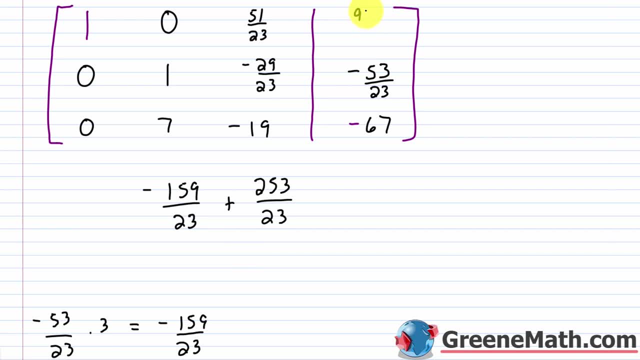 159 over 24.. So this would be 94 over 23.. And now I want a 0 here, So I can multiply row 2 by negative 7, add the result to row 3.. So 0 times negative, 7 is 0.. 1 times negative, 7 is negative. 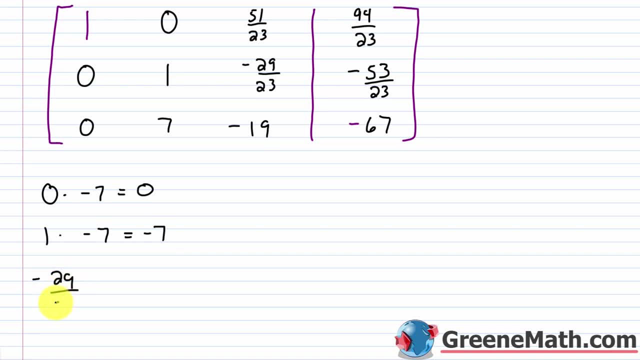 7. Negative: 29 over 23 times negative. 7 would be 1. We know it's positive. And 29 times 7 would be 203. So this would be 203 over 23.. And then we look at negative 53. 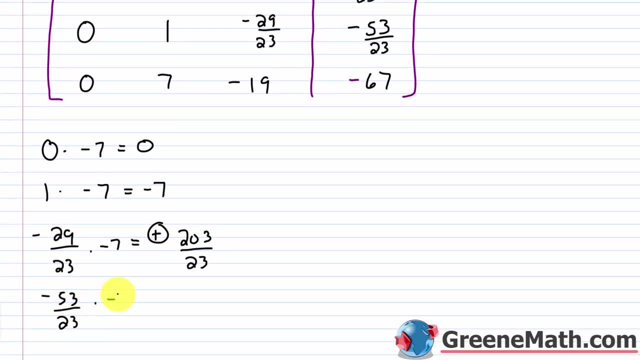 over 23, multiplied by negative 7.. Again, we know it's positive: 7 times 53 is 371.. So it'd be 371 over 23.. All right, So now I want to do my addition: 0 plus 0 is 0.. Negative 7 plus 7 is 0.. 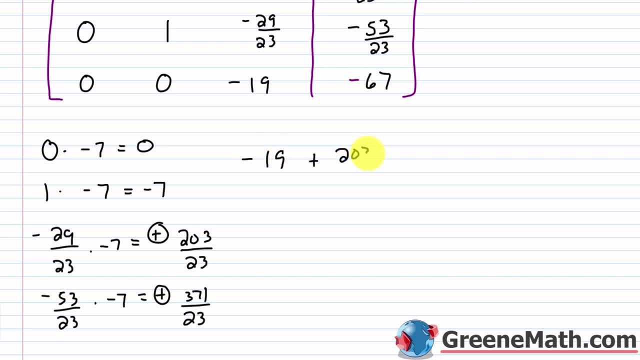 Negative 19.. Negative 19 plus 203 over 23.. So if I get a common denominator here, negative 19 times 23 is negative 437.. So this would be negative 437 over 23.. Negative 437 plus 203 would be. 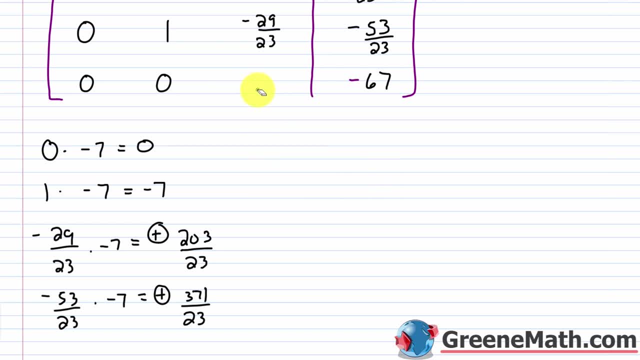 negative 234.. So you would have negative 234 over 23.. All right, So let's erase these, And I've got one more to do, So I want to do negative 67 plus 371 over 23.. Negative 67 times. 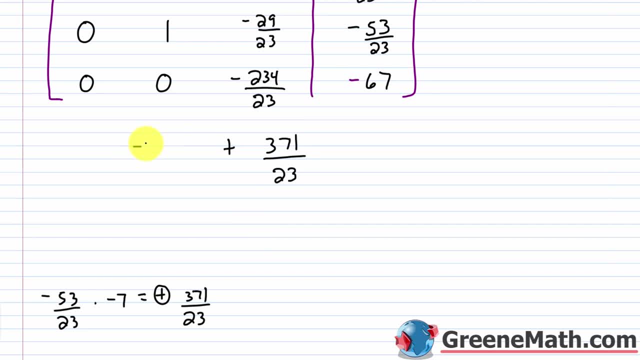 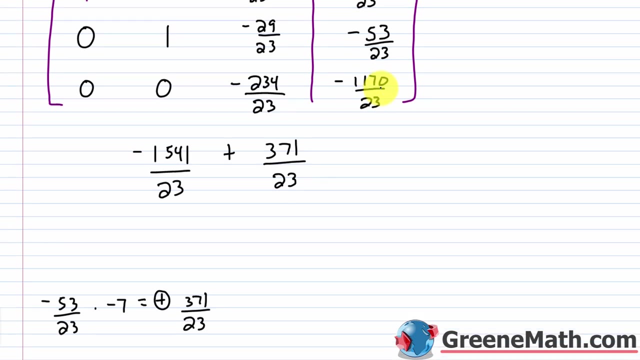 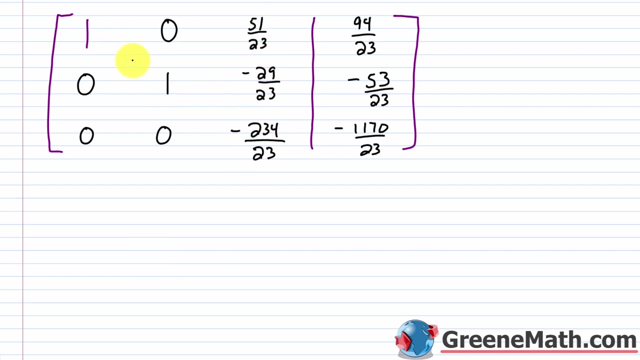 23 would give me negative 1,541.. And then this is over 23.. So negative 1,541 plus 371 would give me negative 1,170 over 23.. This is one bland part of our formula. Let's start our notion of thinking in this way by propagating these stoichiometric properties. 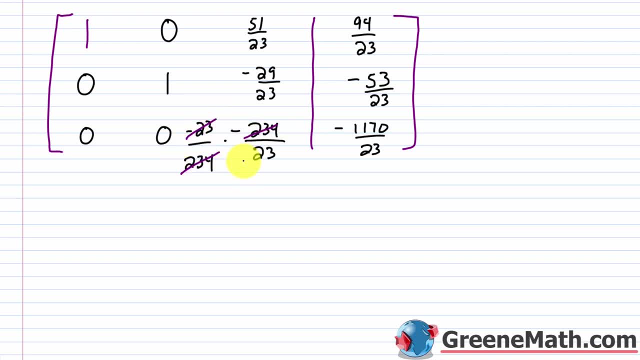 Let's start over. Oh my gosh, There you go, There you go, You've run it, You've done it already. That's what I'm talking about this. So everything cancels and just becomes a 1.. So that's a 1.. Now the next one: negative 1170. 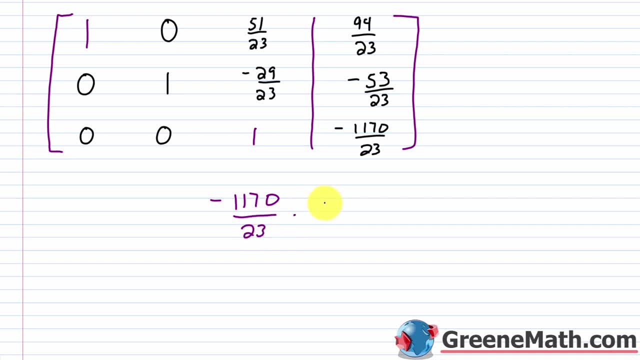 over 23, multiplied by that negative 23 over 234.. It's obvious that the negatives cancel. It's obvious that the 23s would cancel. But what is 1170 divided by 234? Well, that's going to give me 5.. So let's erase this and put a 5 here, So we know what z is at this point. z is going to be: 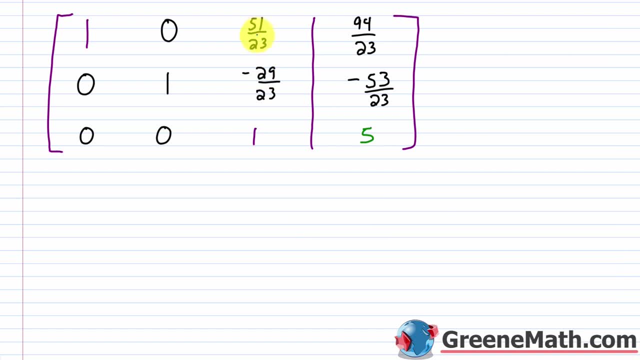 equal to 5.. But let's make this a 0 and this a 0 so we can find out what x and y are. So to make this a 0, I can multiply row 3 by 29 over 23 and add it to row 2.. So I know that multiplication. 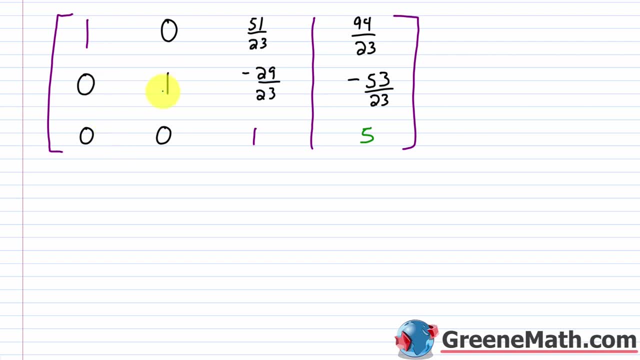 by 0 gives me 0, and adding 0 doesn't change anything. So this one and this one would be unaffected. I only really have to do it for these two. So I would do 1 times 29 over 23.. This equals 29 over 23.. And if I had 29 over 23,, with negative 29 over 23,, I would get 0. 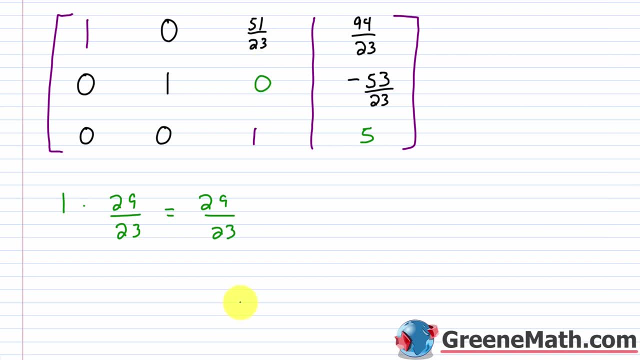 That's easy. The next thing I would want to do is multiply 5 times 29 over 23.. And that would give me 145 over 23.. So this right here, I would add: So 145 over 23,, 145 over 23,, plus negative 53 over 23.. What's that going to give me? Well, it's going to give me. 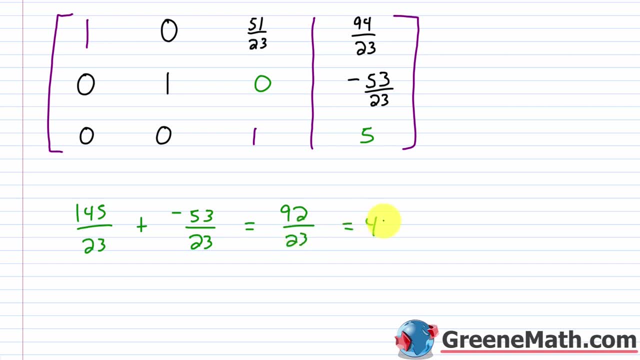 92 over 23,, which is equal to 4.. So this is a 4.. So now I know that z is 5,, y is 4.. So let's continue and figure out what x is. Let's erase this. So how can I make this? 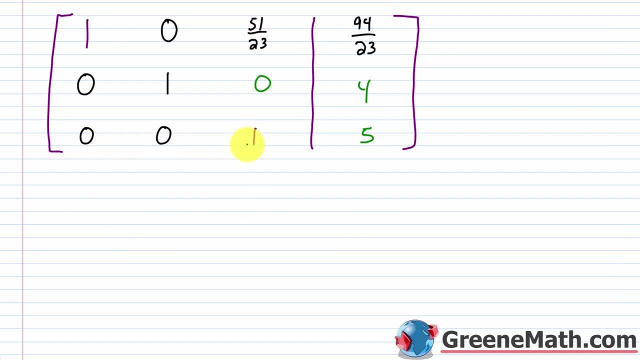 into a 0?? Well, I can multiply row 3 by negative 51 over 23,. add the result to row 1.. All right, I already know, if I multiplied row 3 here by negative 51 over 23,, that the result from this: 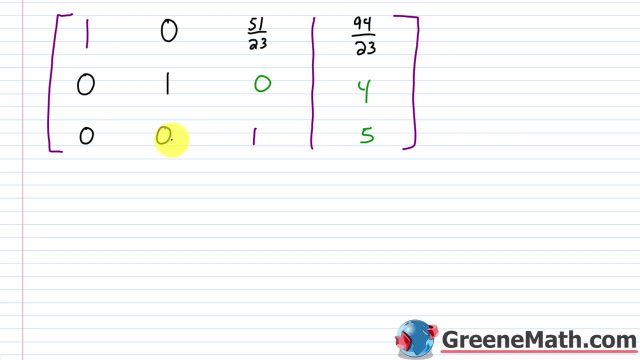 would be 0 and this would be 0. If I add 0 to a number, it remains unchanged, So this one and this one will be unaffected. I would take 1 and multiply it by negative 51 over 23 and get negative. 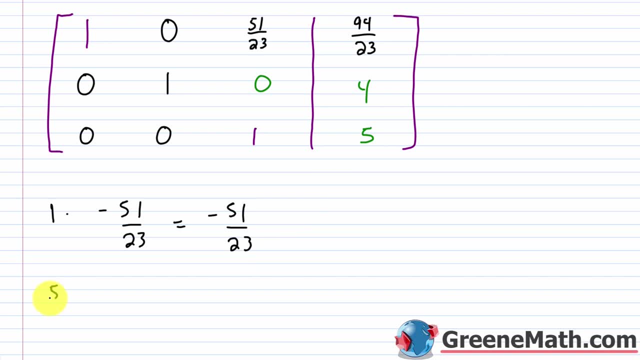 51 over 23. And I would multiply 5 by negative 51 over 23. And I would get negative 255 over 23.. Now, negative 51 over 23 plus 51 over 23,. that's 0. It's pretty easy. So this is gone. 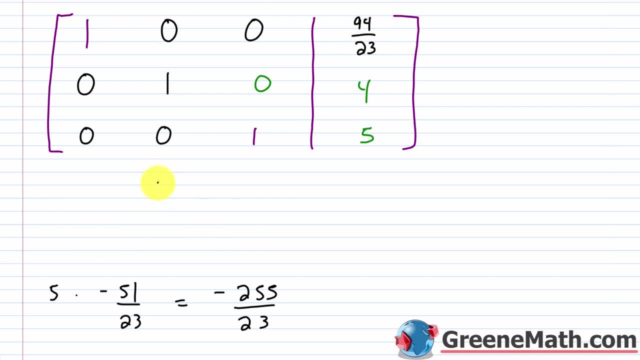 I just need to figure this one out. So I'd have 94 over 23 plus negative 255 over 23.. So this equals negative 161 over 23.. So if I divide negative 161 by 23,, I will get negative 7.. 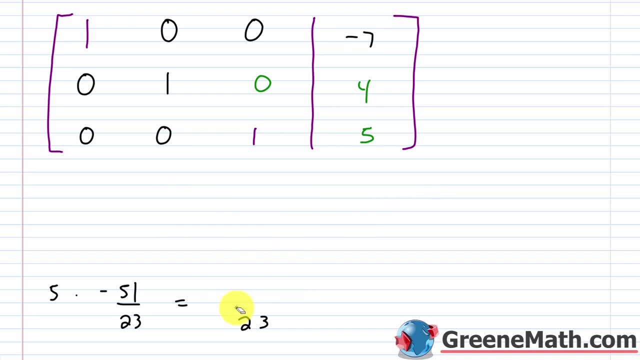 So we're finally done, And I know it takes a long time, especially when you're new to this, But once you kind of get good, you can kind of skip a few things here and there, Some of the calculations like what I just 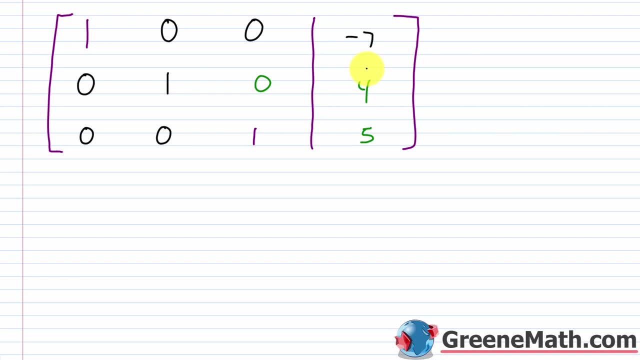 did in the last one. you can do that over and over again And it shortens your time. This really is faster than if you're working with the traditional method. So now that this is in reduced row echelon form, I know that 1x or x is equal to negative 7.. So x is equal to negative 7.. 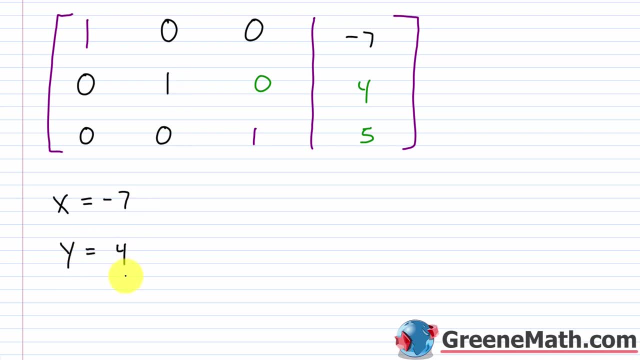 I know 1y or y is equal to 4.. And I know 1z or z is equal to 4.. And I know 1y or z is equal to 4.. And I know 1z or z is equal to 5.. So as an ordered triple, this is negative: 7, 4, 5.. So that's your. 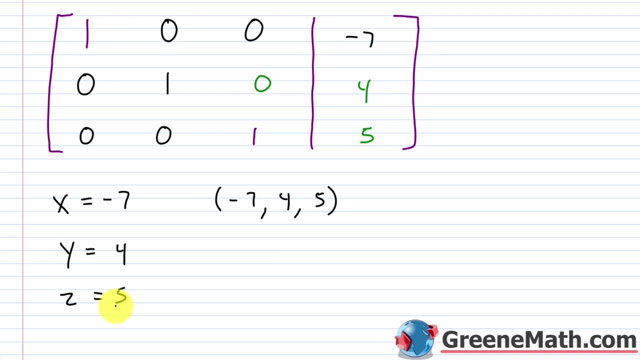 solution for the system. Again, if you want to stop the video at this point, check it in the original system. You'll verify that again. x is negative 7,, y is 4, and z is 5.. Hello and welcome. 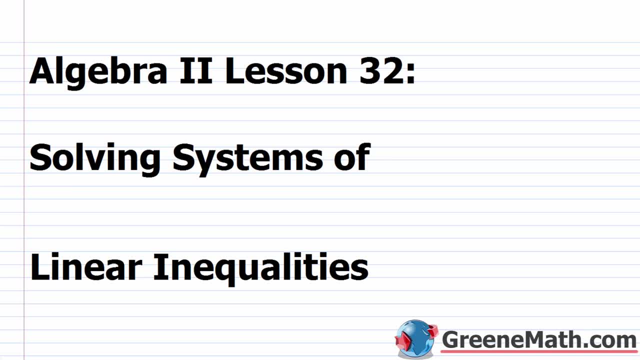 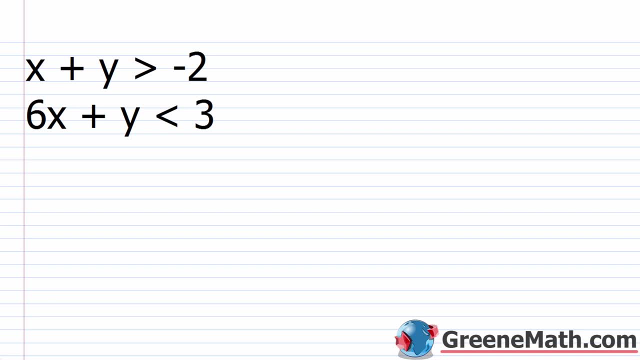 to Algebra 2, Lesson 32.. In this video, we're going to learn about solving systems of linear inequalities. So, now that we've finished talking about linear inequalities, we're going to talk about solving systems of linear equations. We talked about two variables, three variables We learned. 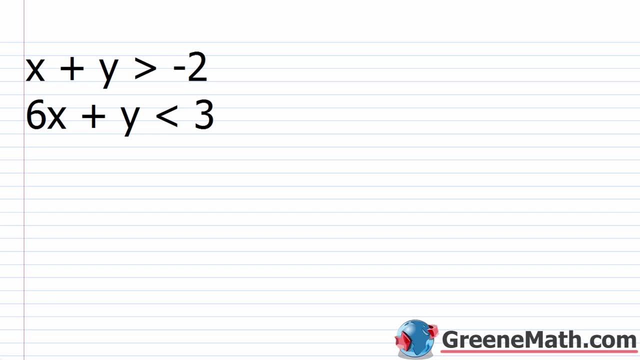 about graphing, substitution, elimination and matrix methods. I want to revisit something that we talked about in Algebra 1.. It's basically the same thing, but I want to make sure that you understand it before we get into college algebra. So when we talk about a system of 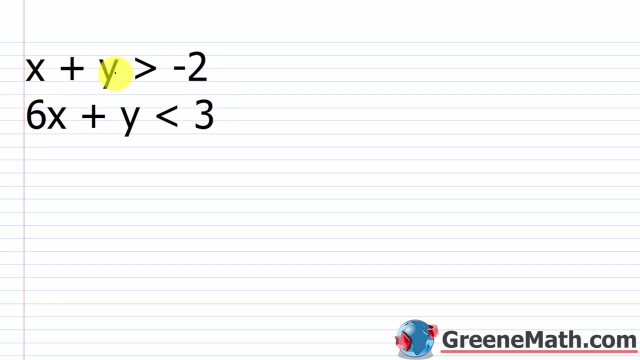 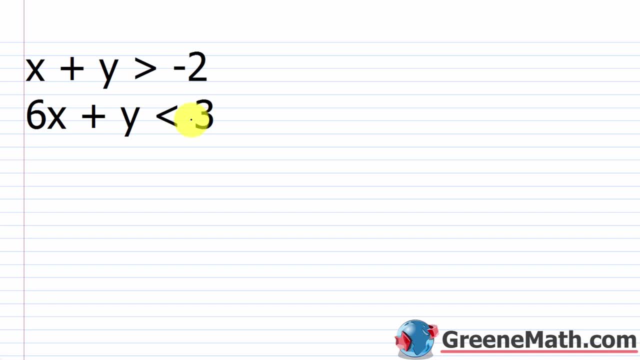 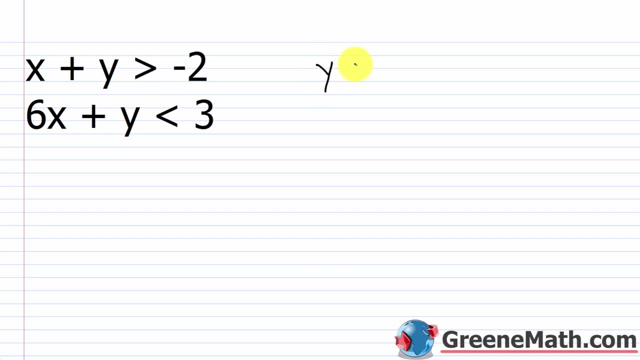 our problem where we would have less than or equal to, And so we can choose y as the root of the station. We can also take the y and z. it will close the tank and compress it as a minus x minus 2. For this one I would subtract 6x away from each side, So y is less than. 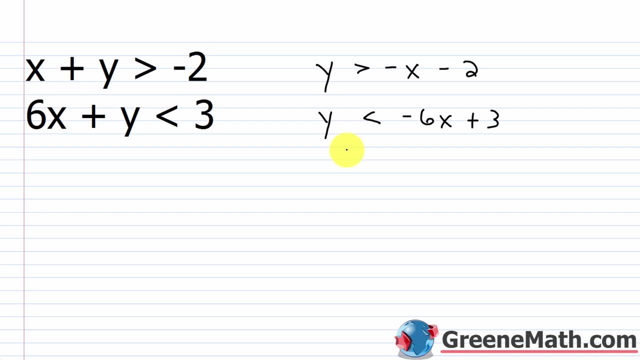 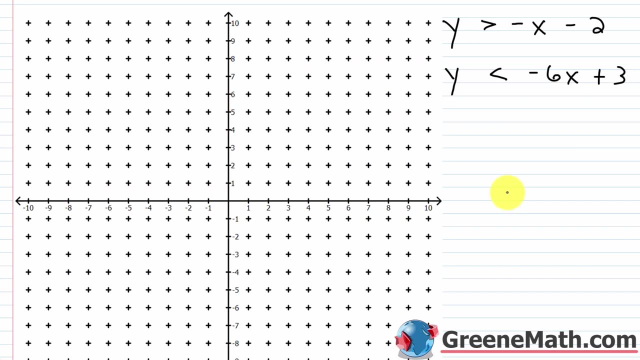 negative 6x plus 3.. So once I have this information, I can just take it to the coordinate plane. Let's just copy it. And so what we're going to do. we know that the boundary line in each case would be what It would be: a broken line, because we have a strict inequality here. y is strictly. 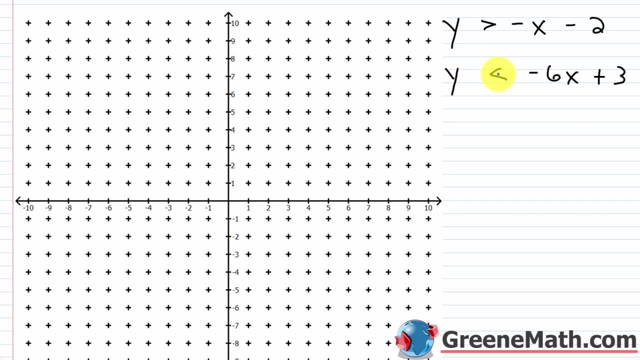 greater than y is strictly less than So in that case the boundary line is not part of your solution. So I think about: y is equal to negative x minus 2.. I graph this with a broken line, So the y-intercept occurs at 0 comma negative 2.. So that's there And my slope is negative 1.. 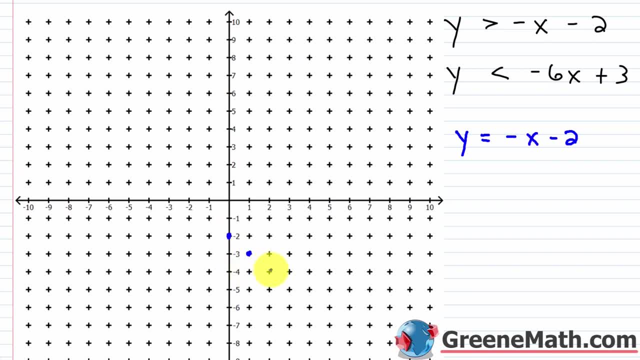 So I'd fall 1, go to the right 1.. Fall 1, go to the right 1.. Or I could rise 1, go to the left 1.. So let's draw a line. Remember, I'm going to break this guy up, So let's just kind of break it up. 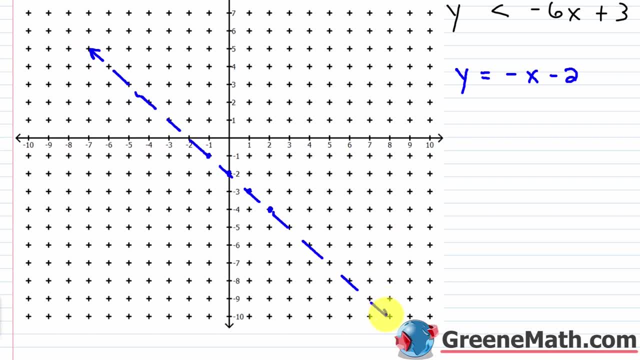 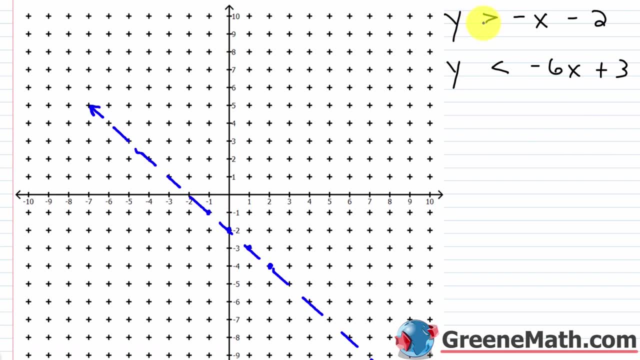 Okay, so that's my line. And where would we shade? You can erase this boundary line. I don't need that anymore. y is greater than, So greater than means I shade above the line. So my solution for this guy right here: I'm shading this way. So all of this. 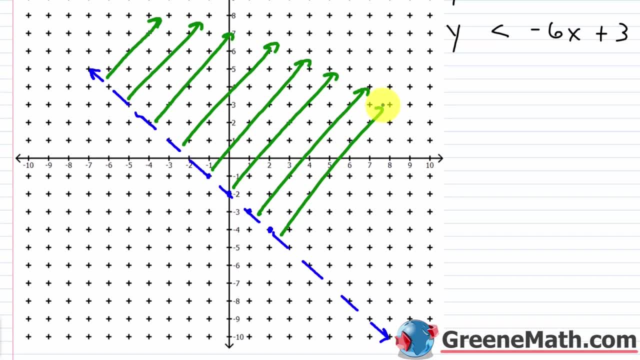 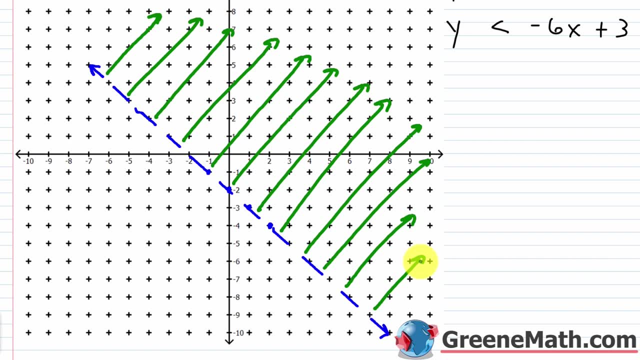 So anything above that line would work as a solution. Now for the second inequality we have: y is less than negative 6x plus 3.. So again another broken or dashed boundary line. So we think about, y is equal to negative 6x plus 3.. The y-intercept occurs at 0 comma 3.. 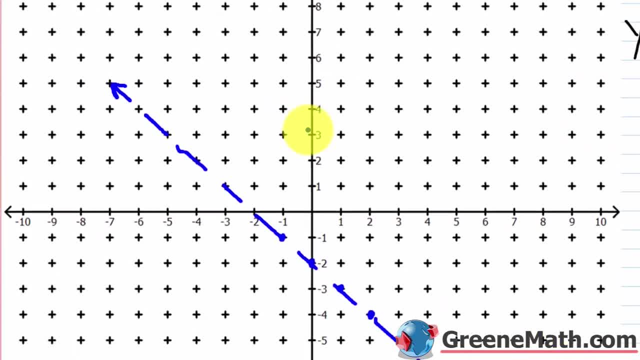 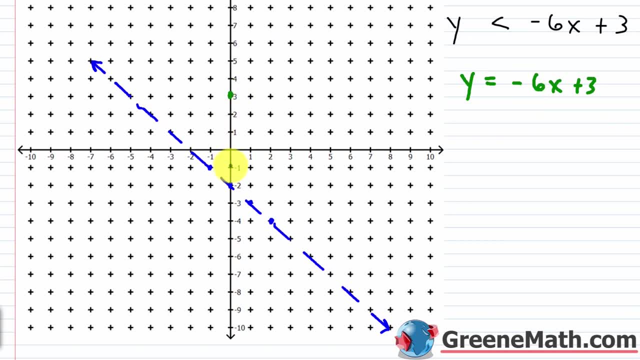 Let me erase this. We know where the solution is for the first one, So it's right here. And then negative 6 is the slope. So fall 6, 1,, 2,, 3,, 4,, 5, 6, go to the right: 1. Fall 6, 1,, 2,, 3,, 4,. 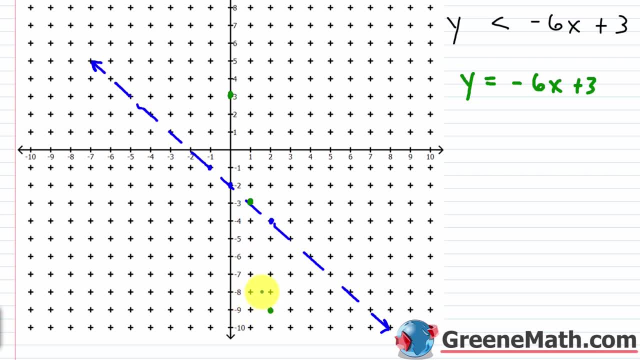 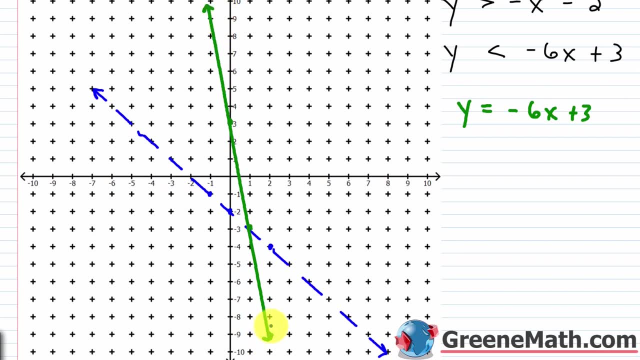 5,, 6, go to the right, 1.. All right, So let's graph that guy. Okay, And again, this has to be broken up. So let me take my eraser out And let me just change the size of it. We'll just take some chunks. out of it. And then negative 6 is the slope. So fall 6,, 1,, 2,, 3,, 4,, 5,, 6, go to the right, 1.. And then negative 6 is the slope. So fall 6, 1,, 2,, 3,, 4,, 5,, 6, go to the right, 1.. And then negative 6 is the slope. 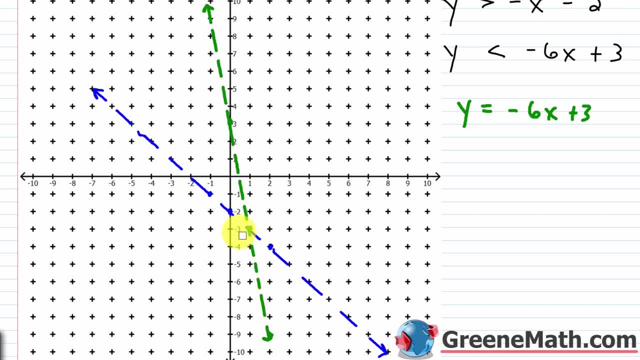 Okay, That's good. Just make sure everybody knows that it's a broken line And we want to shade below this line. So if I'm shading this way here, below the line, and I'm shading above the line here, let me shade this one in black. So this was shaded. 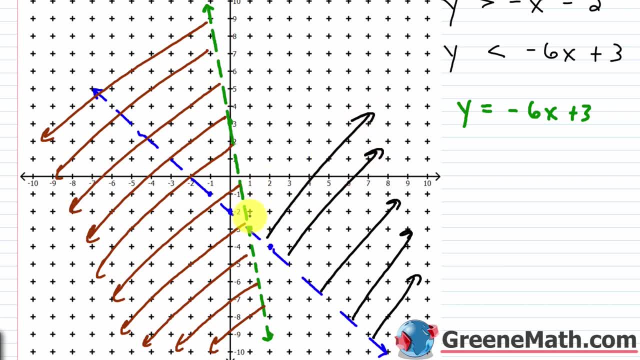 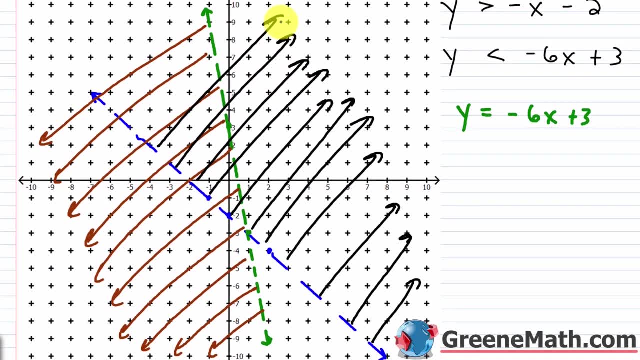 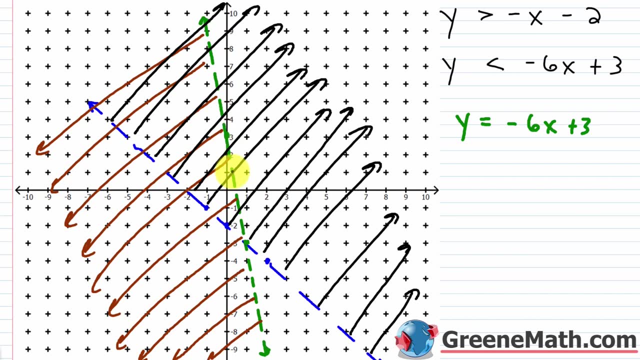 above the line. So if I'm shading this way here below the line and I'm shading above the line, Okay, That's good enough. So anywhere that is below this green line but also above the blue line would work as a solution for the system. So let me kind of get a highlighter going. I'll 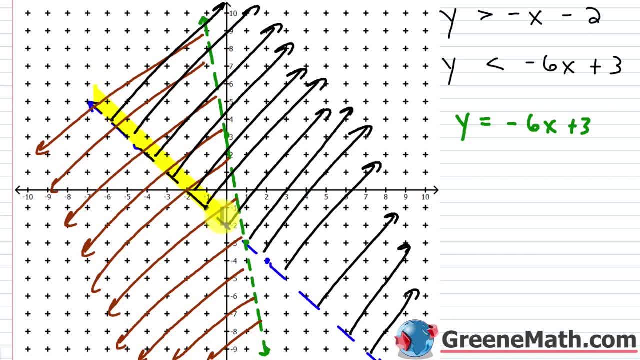 highlight this as best I can. Okay, Went over the line a little bit, but I think you get the idea. Anything above the blue line and below the green line, Okay, Anything that fits that criteria. So it's this area of the coordinate plane here. All right, Let's take a look at the next example. 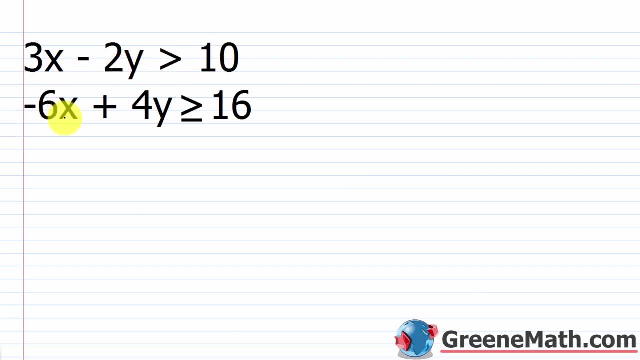 So we have: 3x minus 2y is greater than 10.. Negative: 6x plus 4y is greater than or equal to 16.. So for this one again, we want to solve each one for y. Let's go ahead and subtract 3x away from. 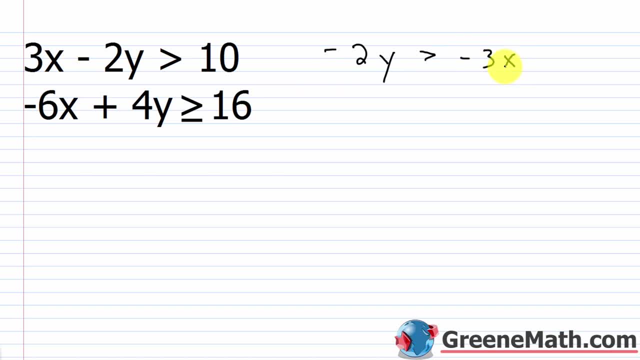 each side of the inequality. So you'd have a negative 3x over here plus 10.. Then I'm going to divide each side of the inequality by negative 2.. Now remember we haven't worked with inequalities in a while. If you divide both sides of an inequality or you multiply both sides of an, 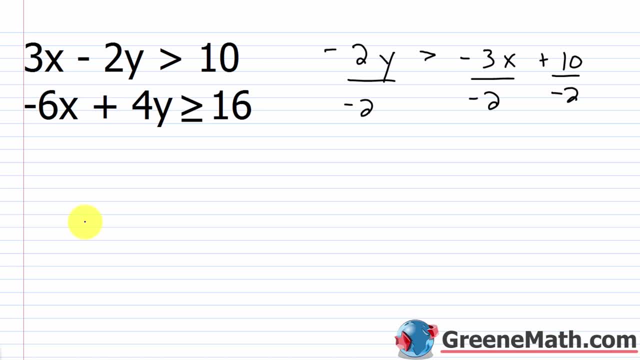 inequality by a negative. what do you have to do? Remember, remember, you have to divide both sides of an inequality. Remember, remember, you have to flip the direction of that inequality symbol. That's going to become a less than So you'd have. y is less than negative, 3 over negative 2.. I can write: 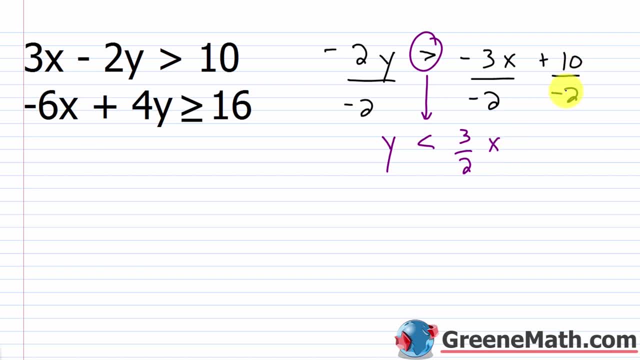 as 3 halves, And then times x, 10 over negative, 2 is negative 5.. So minus 5.. So that one is y is less than 3 halves x minus 5.. For this one, what am I going to do? I can add 6x to each side, So 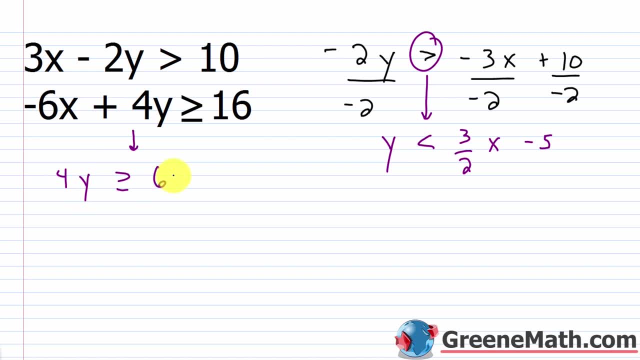 I'd have: 4y is greater than or equal to 6x Plus 16.. We can then divide both sides by 4.. And what are we going to have? This will cancel. with this, I'll have y is greater than or equal to 6 over 4.. Each is divisible by 2.. 6 divided by 2 is: 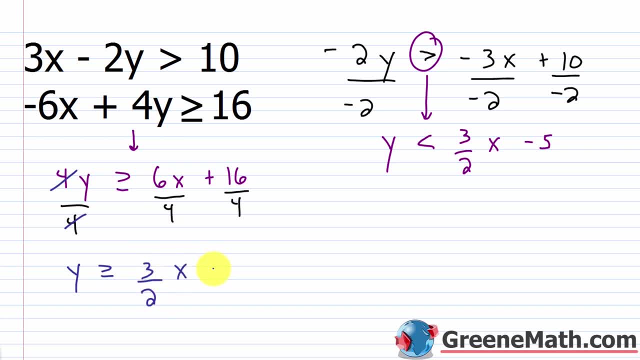 3.. 4 divided by 2 is 2.. So 3 halves x plus 16 over 4 is 4.. So let's write this, as y is greater than or equal to 3 halves x plus 4.. Now 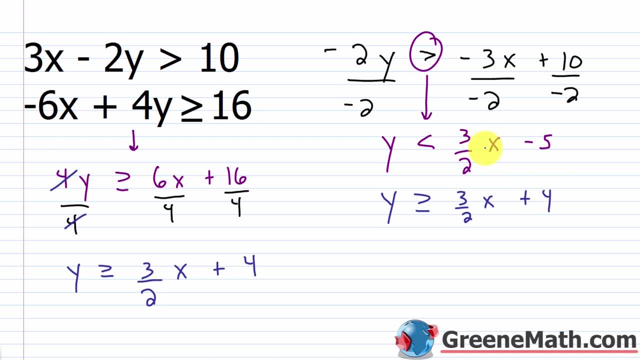 what do we see here before we do anything? Same slope, different y intercepts. Now think about this a little bit more. This is a less than. Y is less than, So I'm going to be shading below this line. This is a greater than or equal to: I'm going to be shading above this. 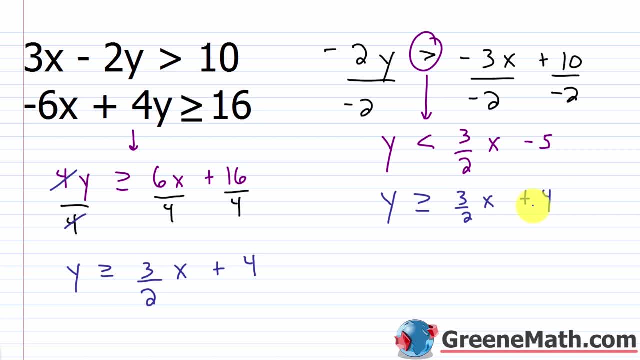 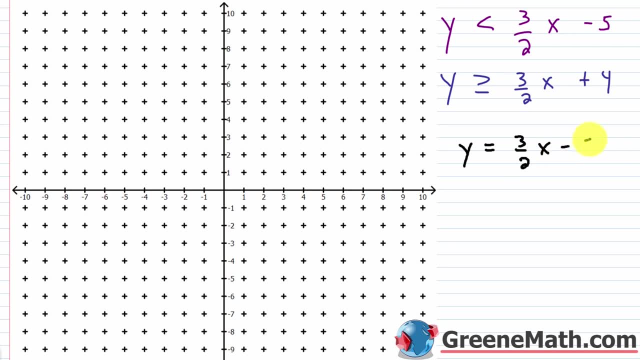 line. Will this system have a solution? No, it will not, And I'm going to show you that. For the first one, you have a strict inequality. So that means your boundary line is going to be a dashed or broken line. 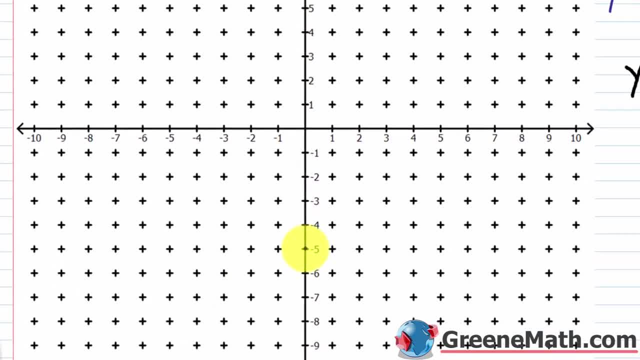 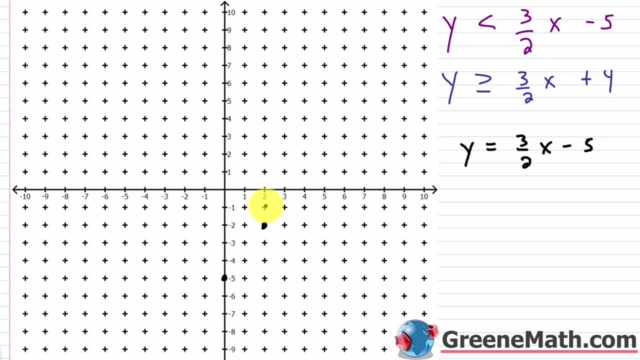 Let's graph: y equals 3 halves x minus 5.. The y intercept occurs at 0 comma, negative 5.. The slope is 3 halves. So up 1,, 2, 3.. To the right: 1, 2.. Up 1, 2, 3.. To the right: 1, 2.. Up 1, 2, 3.. To the 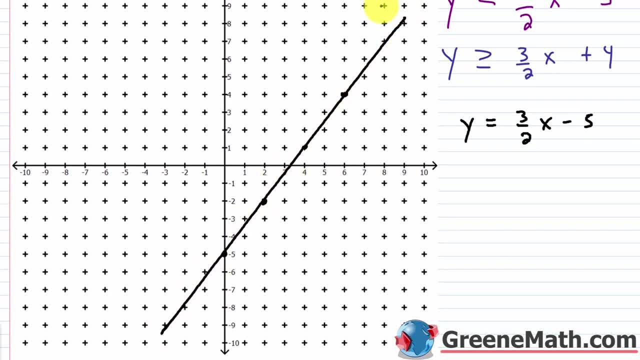 right 1, 2.. And this is supposed to be a broken up line, because this is a strict inequality here. So let's get our eraser out, Take some pieces out of this Again, just enough to make it clear that, hey, this is a dashed line. 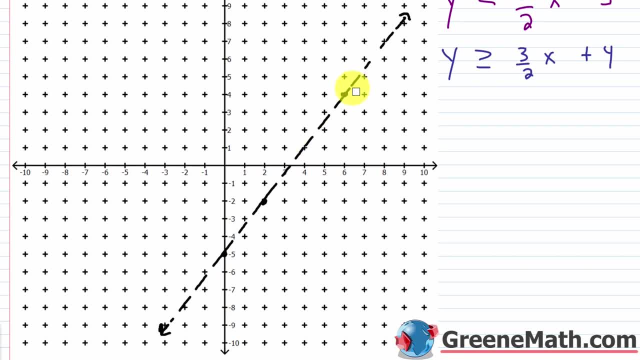 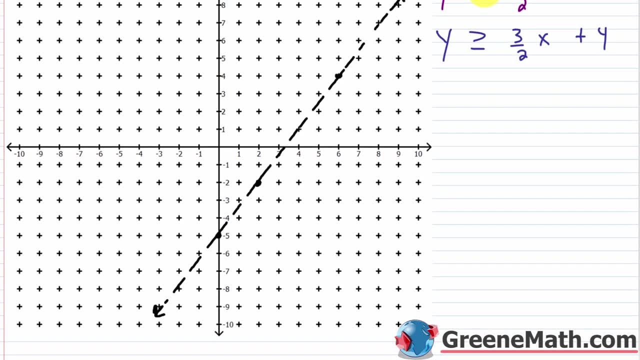 The line is not part of the solution. That's all you need to do, Okay? So I think that's obvious. All right. So the next thing is it's a less than So. that means I would be shading below the line, So I would shade in this direction. 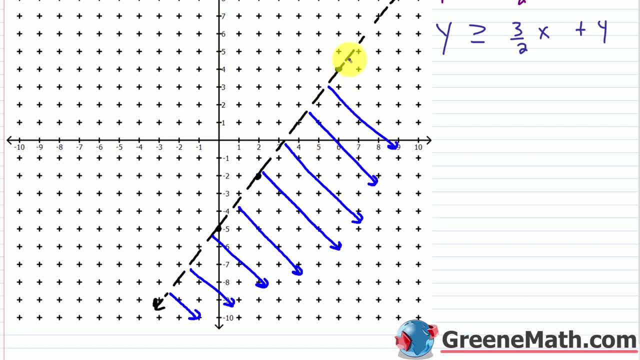 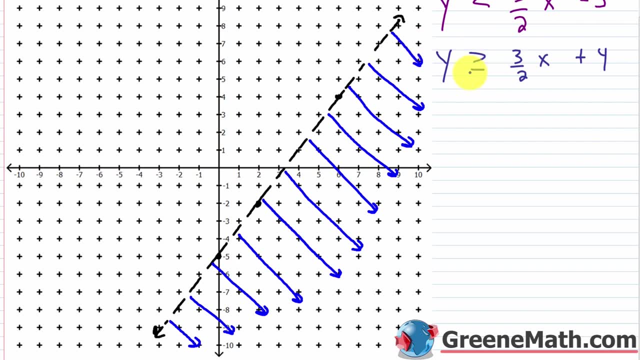 Okay, Now for the next one. I have a non-strict inequality. So that means the boundary line is going to be solid. because the boundary line in this case is part of the solution, Y could be greater than, or y could also be equal to 3 halves x plus 4.. So for that or equals to: 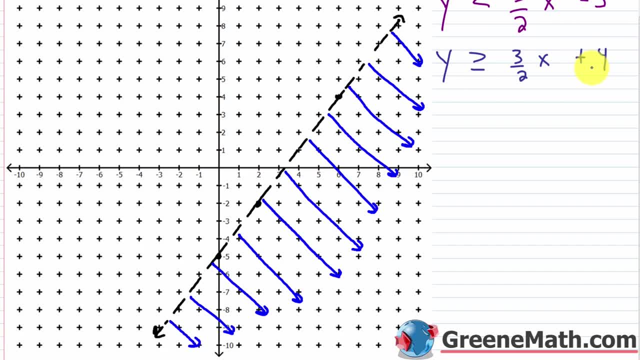 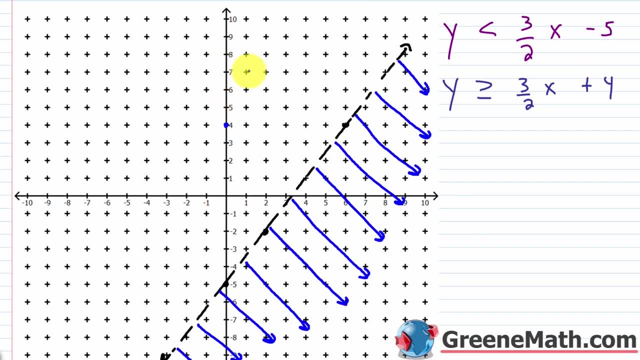 you have to have a solid boundary line. So my y intercept here occurs at 0, 4.. My slope is again 3 halves. So up 3, 1, 2, 3, to the right, 1, 2.. Up 3, 1, 2, 3, to the right. 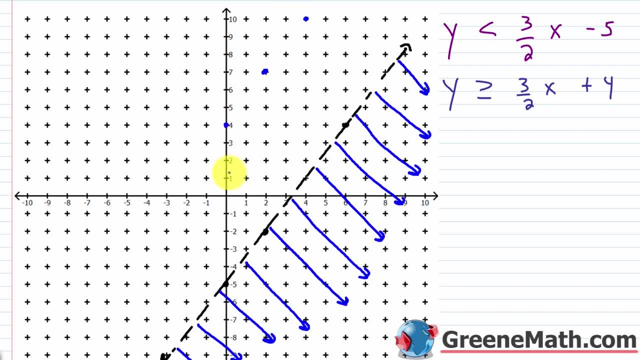 1, 2.. Or I could go down 3, 1, 2,, 3, to the left, 1, 2. Down 3, 1, 2,, 3, to the left, 1, 2.. 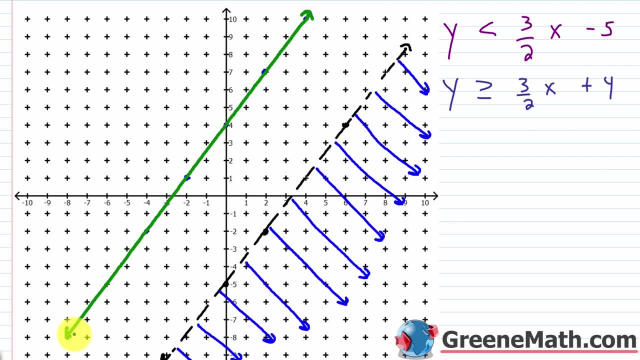 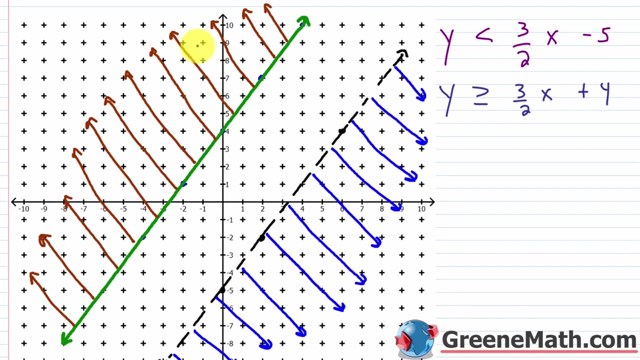 Okay, Now this is a greater than or equal to, So I would shade above the line. So I'm going to shade in this direction. Now, is there any area of the coordinate plane that satisfies both? No, Below this line satisfies. 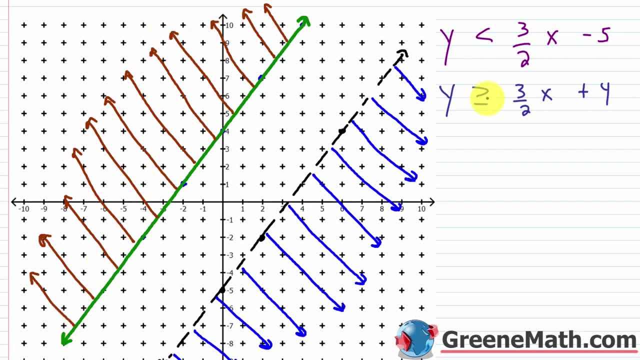 the first one, The line in above the line, satisfies the second. There's no area of overlap, So there's no solution. There's no solution here And again. we found that out right away, that we're going to have the same slope but different y intercepts. 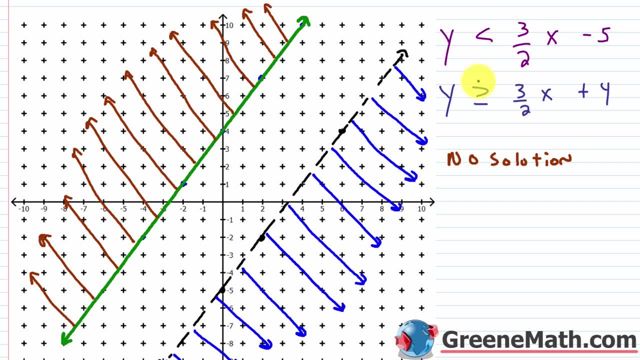 And then we investigated further and we looked at the symbols. We knew this one was a less than and this was a greater than or equal to. So we knew this was going to be the scenario where we're going to come across right, Where there'd be no overlap And so we wouldn't have 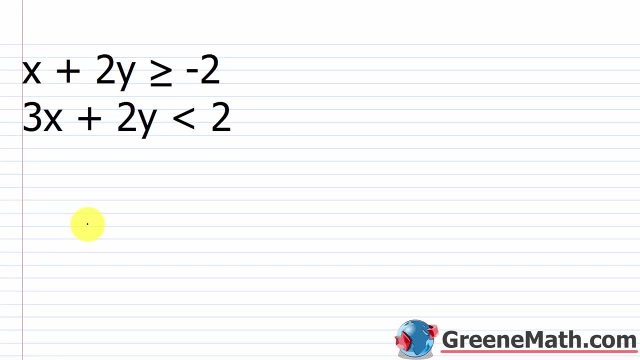 a solution All right For the next system we're going to look at. we have: x plus 2y is greater than or equal to negative 2.. We have 3x plus 2y is less than 2.. We have 2y is greater than. 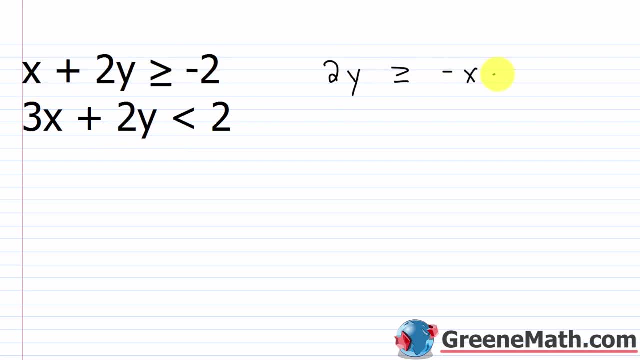 or equal to Subtract x away. So negative x minus 2.. And then we would divide both sides by 2.. So that would give me y is greater than or equal to. You'd put negative 1, half x minus 1.. 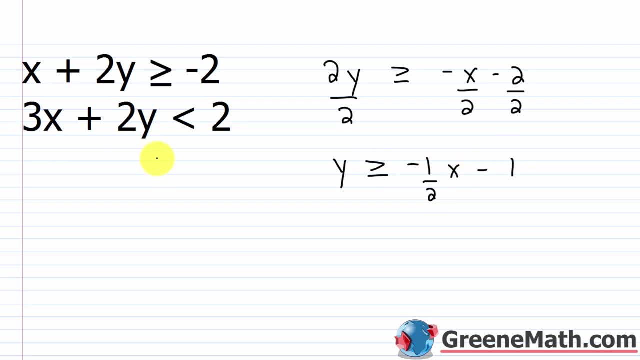 Now for this guy right here. let's subtract 3x away from each side of the inequality. You will have 2y is less than negative, 3x plus 2.. Let's divide both sides by 2. You'll have: y is less than negative, 3 halves x plus 1.. So y is less than negative, 3 halves x plus. 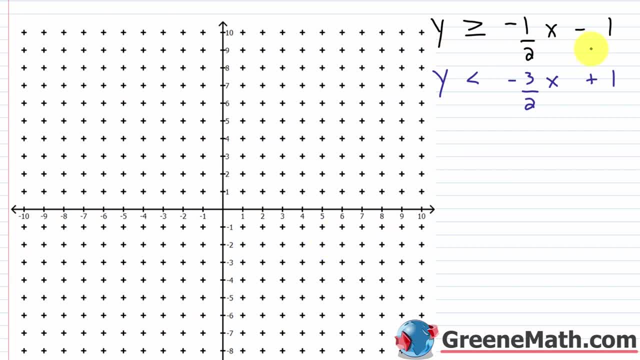 1.. If I look at this first one here, the boundary line will be solid. I'm basically going to graph: y equals negative 1 half, x minus 1, so the y intercept would occur at 0 comma negative 1, And the slope is negative 1 half, so down 1 to the right, 2. 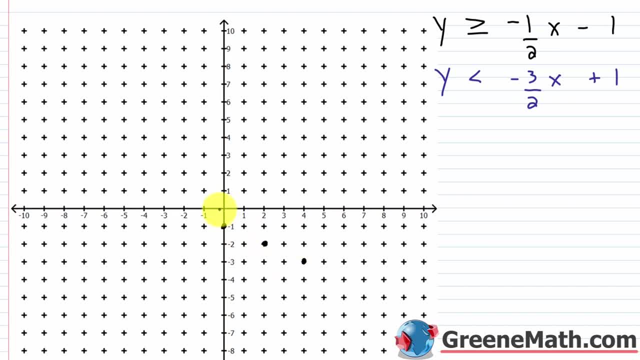 Down 1 to the right, 2. or up 1 to the left, 2. up 1 to the left, 2. All right, so this is a greater than or equal to, so I'm going to shade above this line, So I would shade everything going this way. 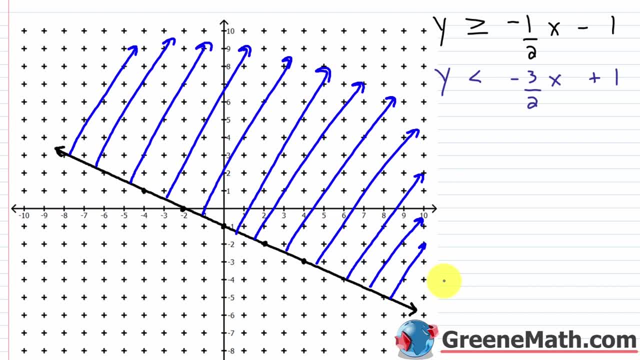 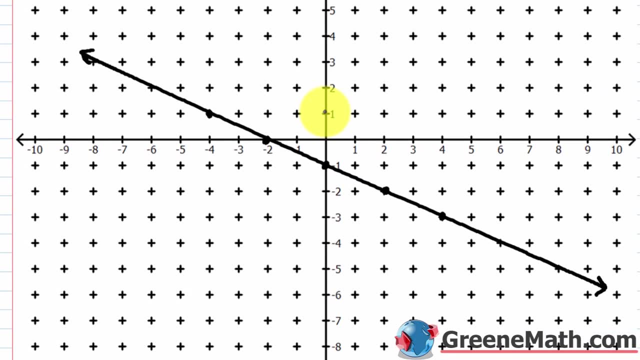 Now for the next guy. I have a dashed boundary line, So I have: y is less than negative 3 halves x plus 1. So I would graph: y equals negative 3 halves x plus 1.. Let me just erase this temporarily. The y intercept occurs at 0 comma 1. 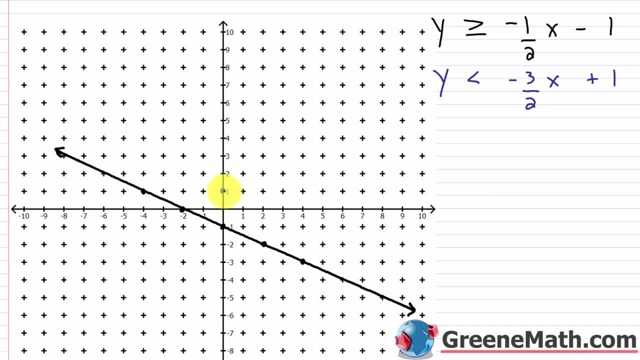 So I would graph: y equals negative 3 halves x plus 1. So I would graph: y equals negative 3 halves x plus 1. That's here The slope is negative 3 halves, So down: 3, 1, 2, 3 to the right: 2, 1, 2 down. 3, 1, 2, 3 to the right: 1, 2. 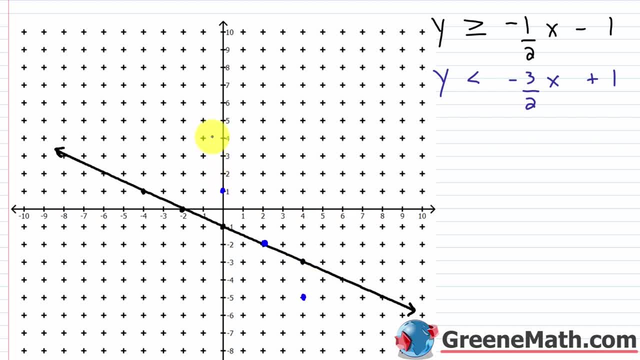 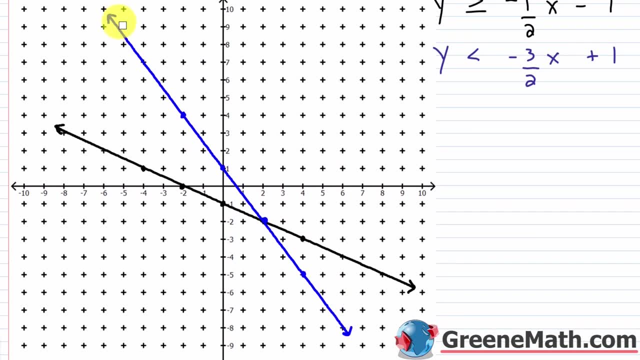 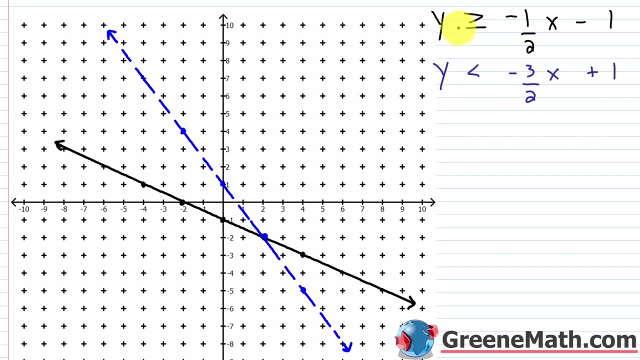 Or I could go up: 3, 1, 2. 3 to the left, 1, 2. All right, so let's break this up a little. eraser. So let me reshade the first one. We had a greater than or equal to. This was the first one here, the line in black: 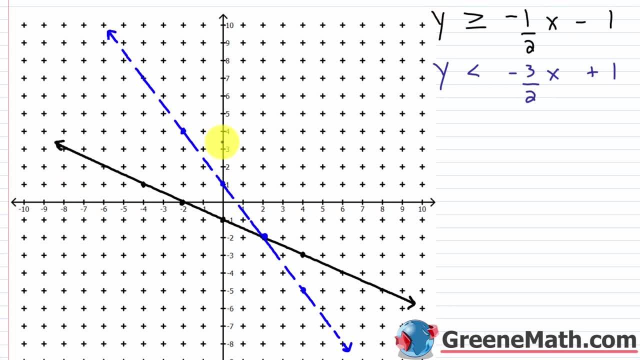 We were supposed to shade above the line. We did, but we had to erase it so we could draw this one. So let me reshade this. so we're shading above the line. Now for the second one. we want to shade below the line. That's a less than. 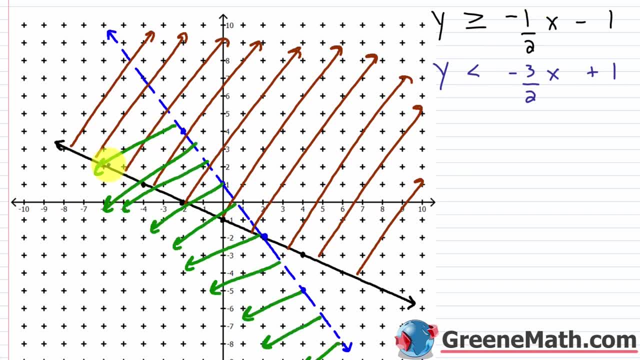 So let's shade this in a green. You can see where it overlaps. So let's shade this in a green. So let's shade this in a green. So anything below the blue line And anything at the black line or above the black line, Anything that fits into that region. 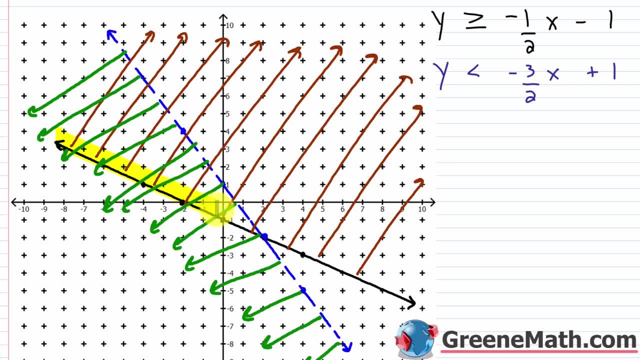 And we gotta highlight it. Well, the black line itself is included here, Up to that point, right there, Up to that point, right there. And then, let me kind of highlight this, The blue line here would not be included Because it's not part of the solution. Okay, And I know I went over it a second time just to be sure. 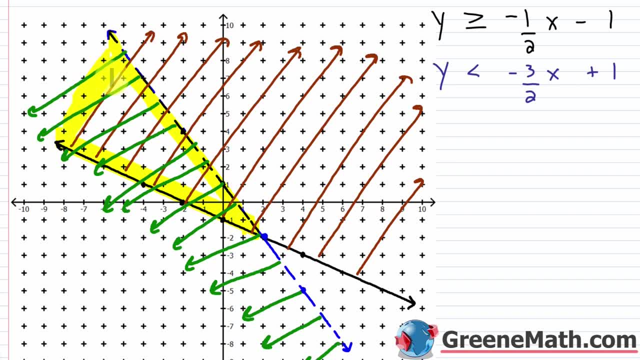 Okay, And I know I went over it a second time just to be sure the line, but just pretend i didn't okay, so i'll shade all this. so that's where the two graphs overlap and this is an infinite area. we continue out here forever and ever and ever, but we just look at a small portion just to get a general idea of where the 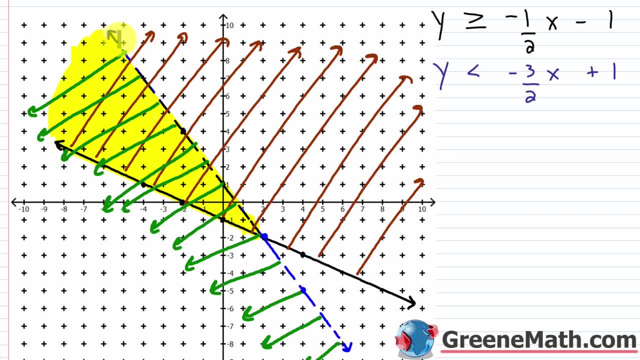 solution for the system would be. so anything below this blue line here, not including that blue line, going down, that's also including the black line, but going up. so anything that i've highlighted in yellow, that region of the graph, would satisfy the system. hello and welcome to algebra 2 lesson. 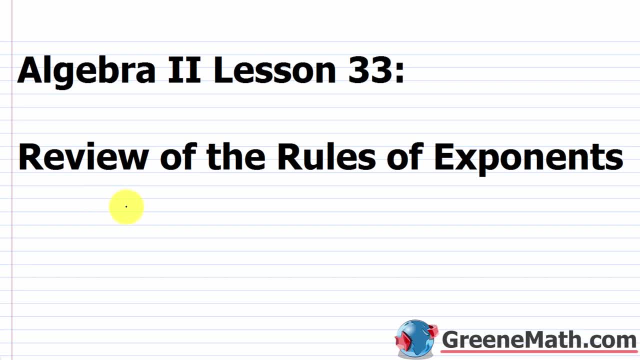 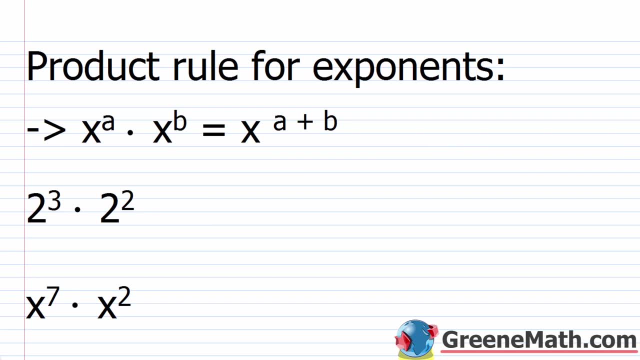 33.. in this video we're going to have a review of the rules of exponents. so i know for the majority of you, you thoroughly covered the rules of exponents when you were in your algebra 1 course. now we're about to start working with polynomials again. 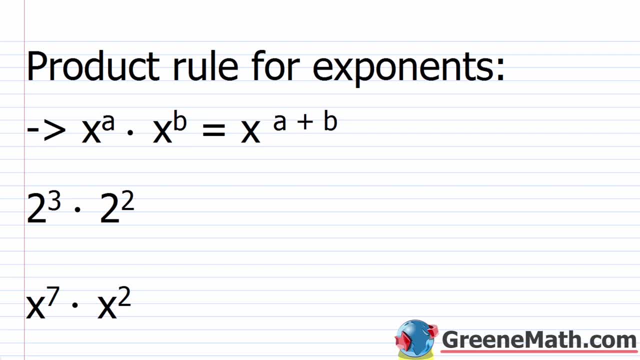 so it's very, very important that we understand the rules of exponents. so that's why we're going to review them in this lesson and then in the next lesson, we'll start working with polynomials again. so the first rule i want to cover is the product rule for exponents: super, super easy to remember. 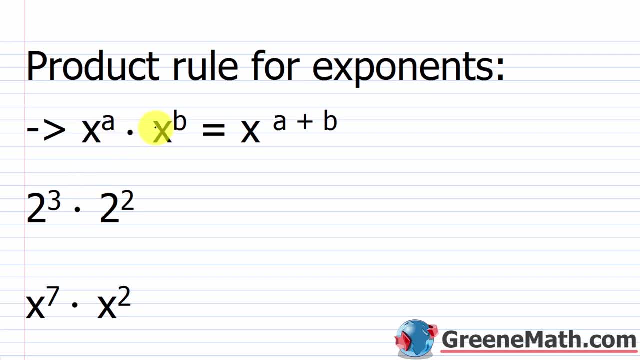 what it says is: if you have like bases and you're multiplying, what you do is you keep the base the same and you add the exponents. so, as an example, we have x to the power of a times x to the power of b. so the base is the same in each case. we have x and we have x. so what we do is we say this is equal to x. 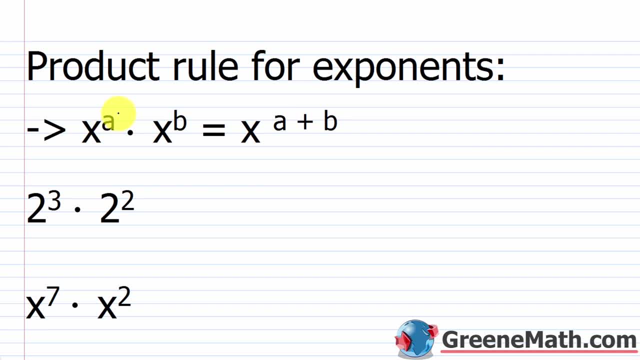 base stays the same and we add the exponents. exponent here is a, so i have a plus the exponent here is b, so i have b, so x to the power of a plus b. and as an example of this we have 2 cubed times 2 squared. so the base in each case is the same. 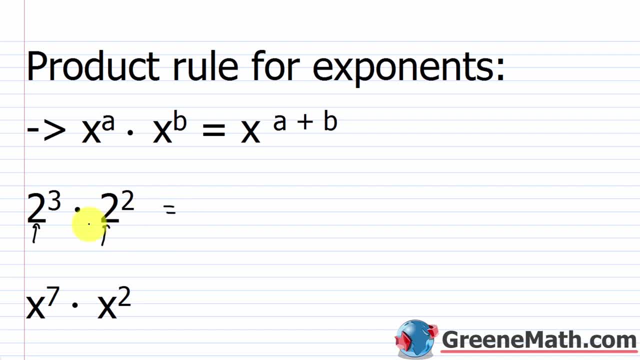 it's a 2 here and it's a 2 here, so i would keep 2 the same and i would add the exponents. i would add 3 plus 2, which would give me 5, so this is 2 to the 5th power. now, when we work with exponents, we 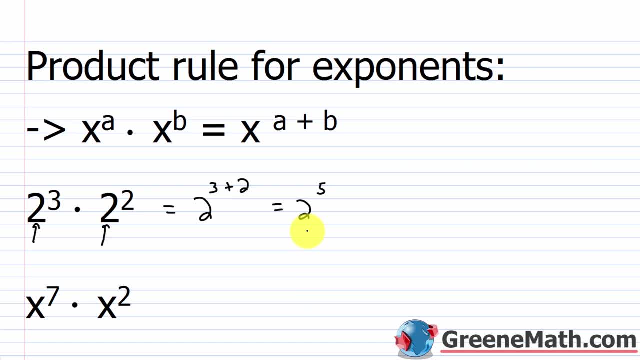 can leave this as 2 to the 5th power because it's nice and convenient, or you could write 32. you can evaluate it if you want. really, if you're in this section on your textbook, a lot of answers will be kept in that form. all right, so let's scroll down a little bit. 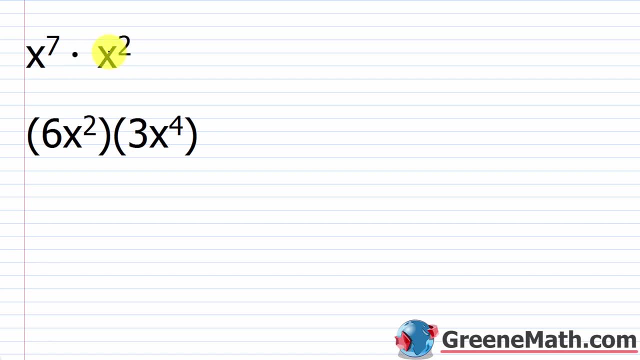 for the next example, we see x to the seventh power times, x squared, so the base x is the same. so I'll keep it the same and I'll add the exponents. Here I have a 7,, here I have a 2.. 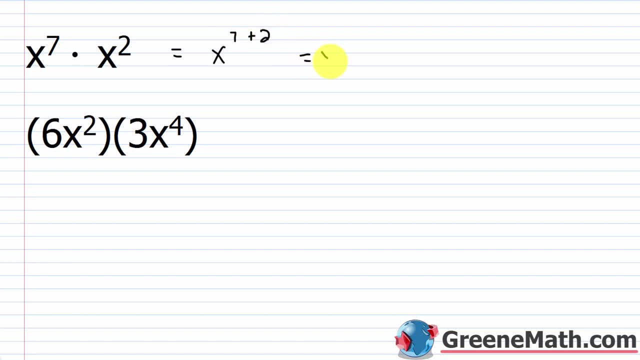 So this would be x to the power of 7 plus 2, which is x to the power of 9.. For the last example, I have 6x squared times 3x to the fourth power. So what I'm going to do is I'm going to write. 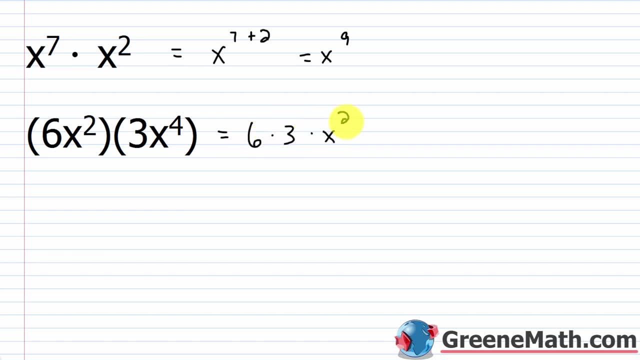 this as 6 times 3 times x squared times x to the fourth power. We know that 6 times 3 is 18, and then x squared times x to the fourth power. We have the same base, that's x, so we keep that. 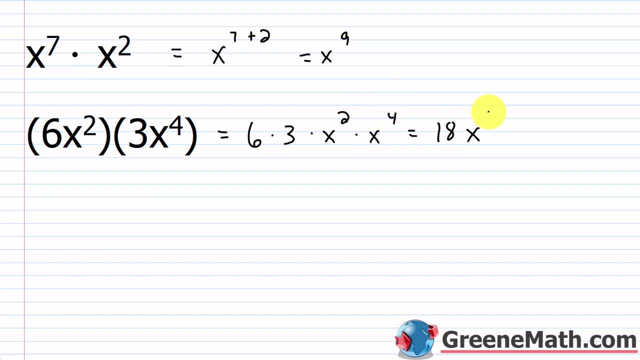 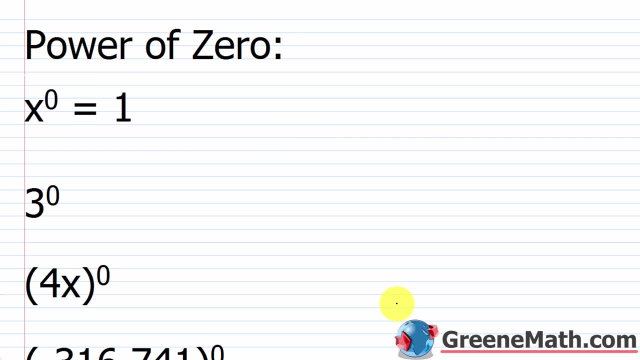 the same, and we add the exponents, 2 plus 4 is 6.. So this would be 18x to the sixth power. All right, so the next rule I want to deal with relates to the power of 0. So what happens when? 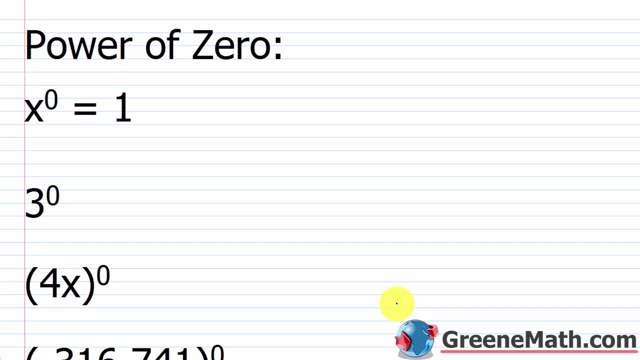 we raise a non-zero value to the power of 0?? Well, it's 1, right? So if I have some x raised to the power of 0, as long as I have a non-zero value to the power of 0, I have a non-zero value to the. 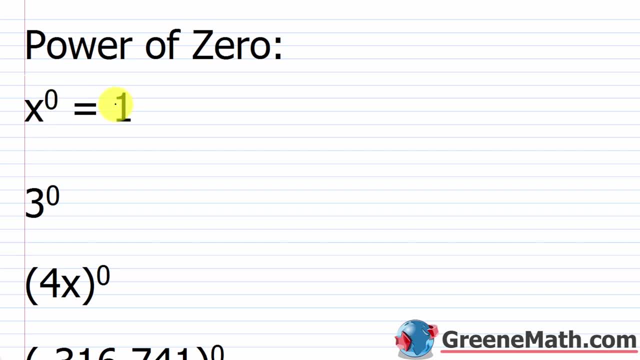 power of 0. So if I have some x raised to the power of 0,, as long as I have a non-zero value to the power of 0,, as long as x is not equal to 0,, the value is always going to be 1.. So it doesn't matter what. 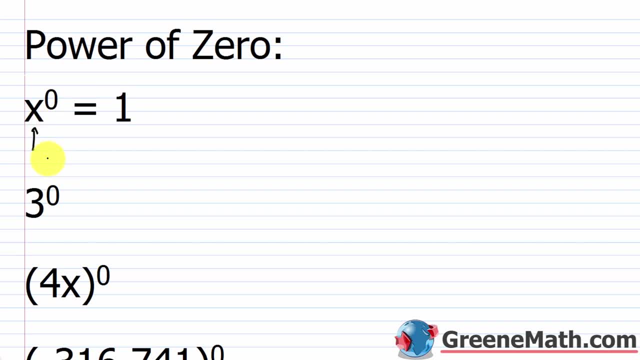 I plug in here for x as long as it's not 0, and let me state that we'll say x does not equal 0,, then the value here is going to be a 1.. So, for example, 3 to the power of 0 is 1.. This whole. 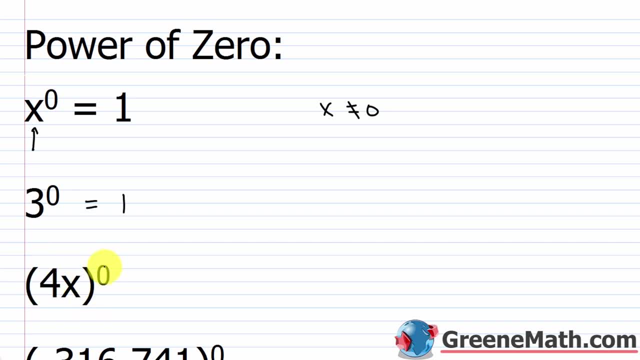 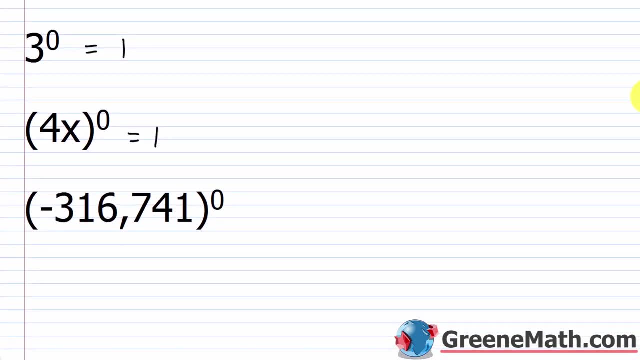 amount 4x or 4 times x- it's in parentheses and it's raised to the power of 0. So this is 1.. Then down here- let me kind of scroll down a little bit- We have negative 316,741 raised to the power of 0. Everything's in parentheses there, So this: 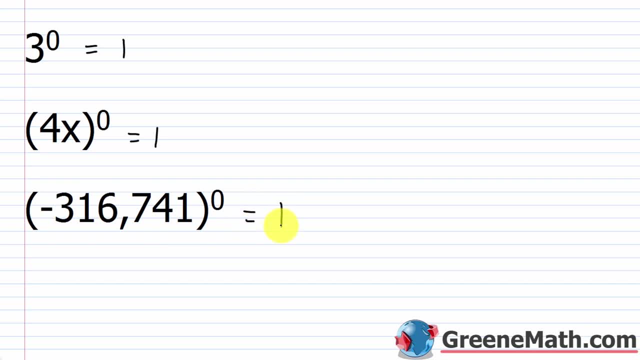 equals 1.. So, again, it doesn't matter what it is. It could be 1 billion, It could be 1 trillion, It could be whatever you want, as long as it's not 0.. When the value is raised to the power of 0,, 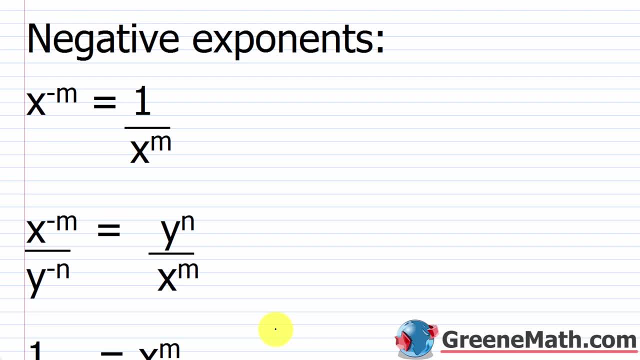 it's equal to 1.. So the next thing we want to talk about would be negative exponents. So what do we do when we run across these? So if I have x to the power of 0, negative m, this is equal to 1 over x to the power of m. So basically, what you're doing here. 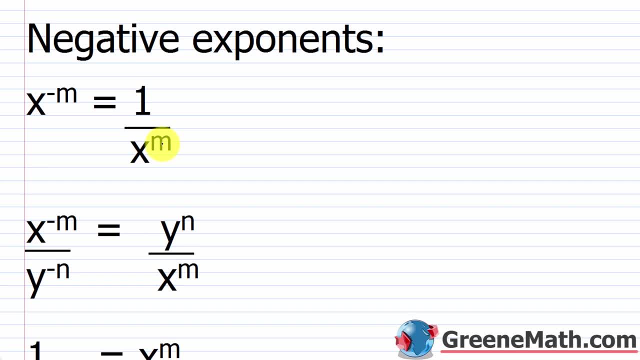 is you're taking the reciprocal of the base and you're making the exponent positive. So the reciprocal of x would be 1 over x. That's how we have 1 over x here And the exponent goes from negative m to positive m. Another way you can kind of think about this: if I have x to the power of, 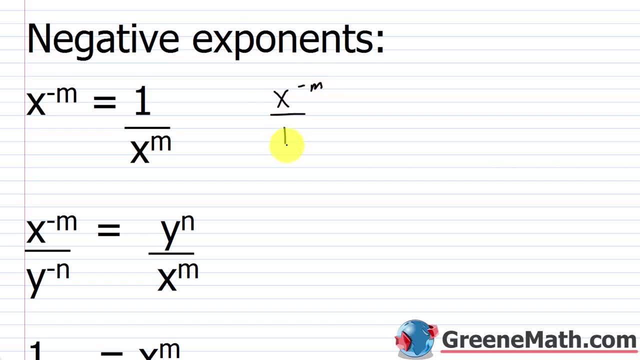 negative m and I just write it over 1.. If I drag something to the power of 0, and I write it over something across the fraction bar, I just have to change the sign of the exponent. So if I drag this across the fraction bar here, what's going to happen is I'm going to have a 1 up here And 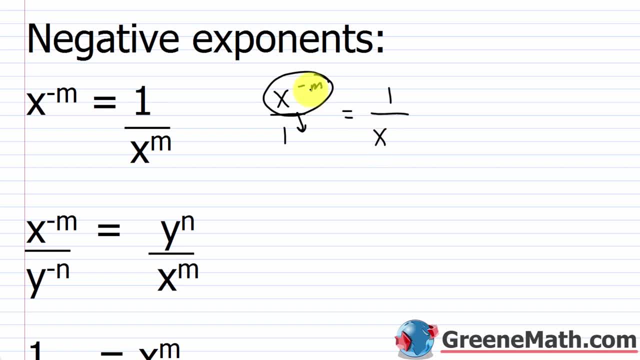 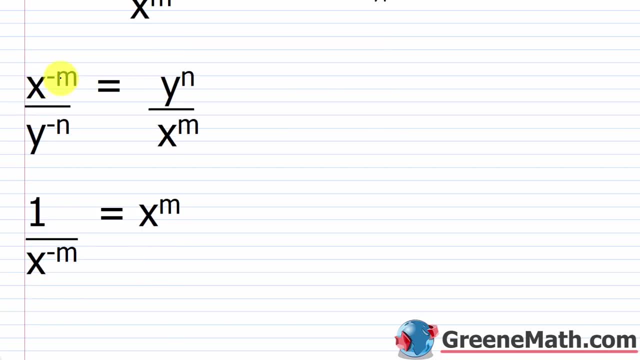 then down here. since I dragged this down, I'd have x raised to. since this was negative, it will now be positive. So here's a perfect example of that. I have x to the power of negative m over y to the power of negative n. As I drag this across the fraction bar. 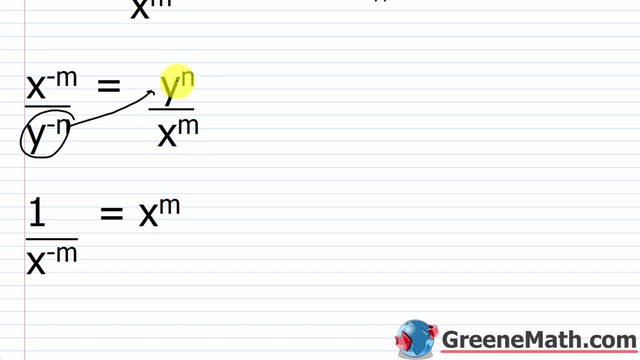 you'll see. here it's in the numerator. y is the same, It's just that the exponent has changed its sign. It goes from negative to positive. Same thing here. x gets dragged across the fraction bar. It's now in the denominator. And notice how the sign on the exponent has changed. Here it's. 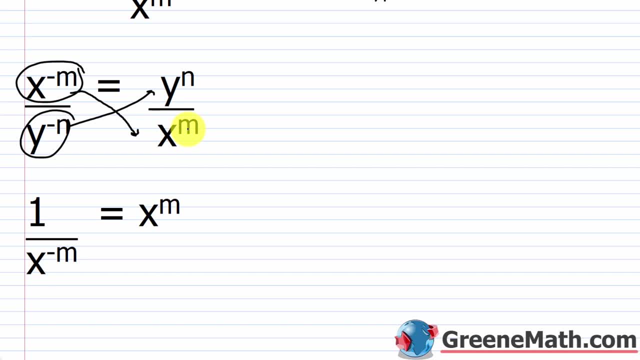 negative, Here it's positive. So if you drag something across the fraction bar, right from numerator to denominator or from denominator to numerator, you just need to change the sign of the exponent. So as an example with some numbers, let's say you had something like 6 to the power of negative 2. And this is 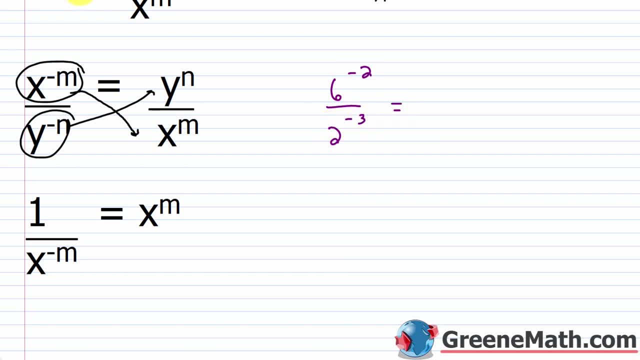 over, let's say, 2 to the power of negative 3.. What we can do is we can take this guy right here, We can bring it into the numerator. We just have to make the exponent positive, So this would be 2 cubed. And then we could take this guy right here, bring it into the denominator. We just 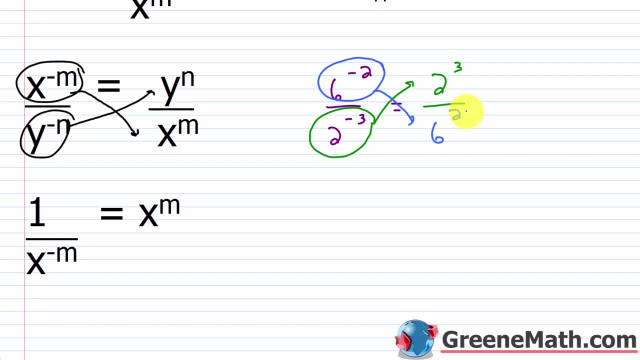 have to make the exponent positive. So that would be 6 squared. You could verify that with a calculator. I can simplify this: 2 cubed is 8.. 6 squared is 36. And we know they have a common factor. This would: 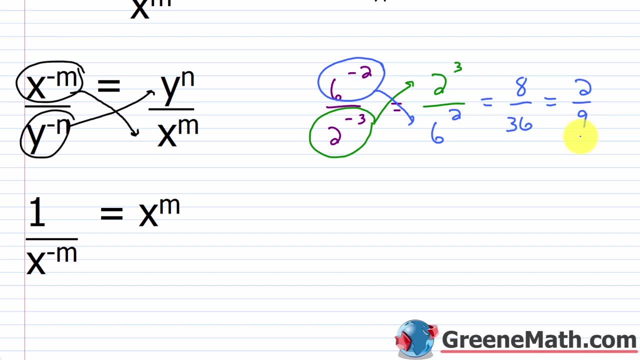 end up being 2 over 9 in its simplest form, And you can punch this up on a calculator and verify. You can do 6 to the power of negative 2, divided by 2 to the power of negative 3.. Now you're going. 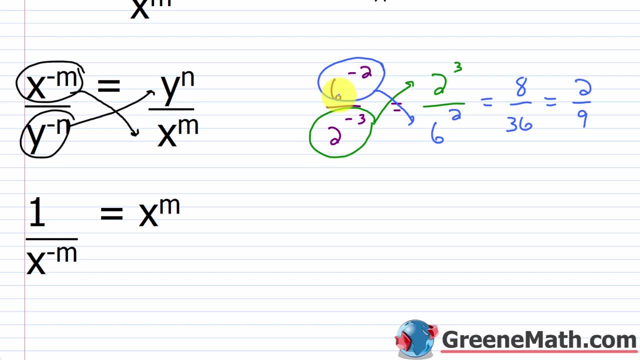 to end up with a decimal, that's 0.2, with the 2 repeating forever and ever and ever. But it just verifies that you have the same answer here. So you can do 6 to the power of negative 2. And you can. 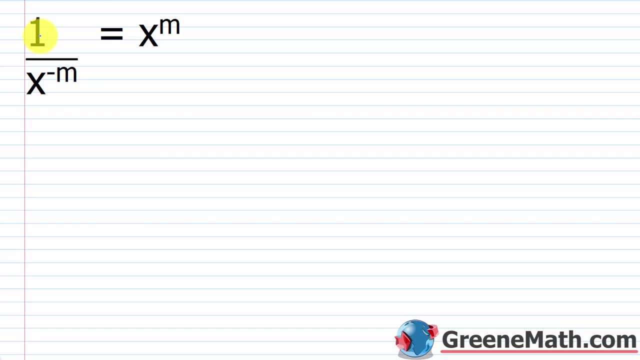 take this guy right here as the fraction 2 ninths. So I also have here 1 over x to the power of negative m is equal to x to the power of m. So if you have 1 over something where that something has a negative exponent, again I can just drag this up into the numerator. I can think about this as: 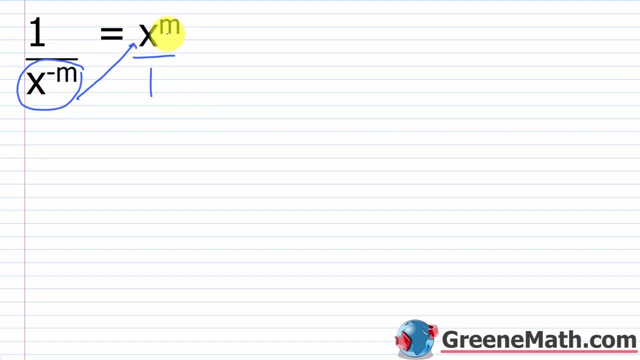 being over 1.. And I can change the sign of the exponent. Another way to think about this kind of a longer way to think about this: if I have 1 over x to the power of negative m, remember, I could take the reciprocal of the base, make the exponent positive. So I could write this: 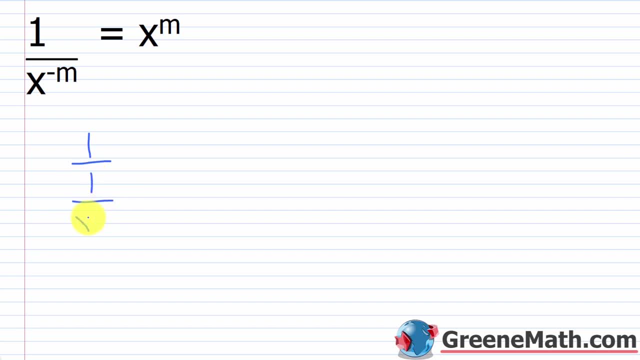 as 1 over 1 over x to the power of m. So if 1 is divided by this fraction, really I could write 1 over 1 divided by 1 over x to the power of m, which turns into 1 over 1 times the reciprocal. 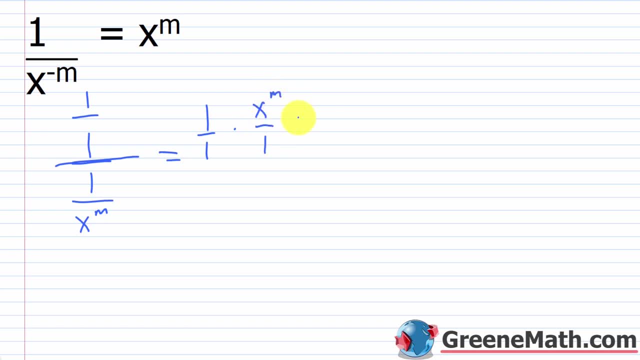 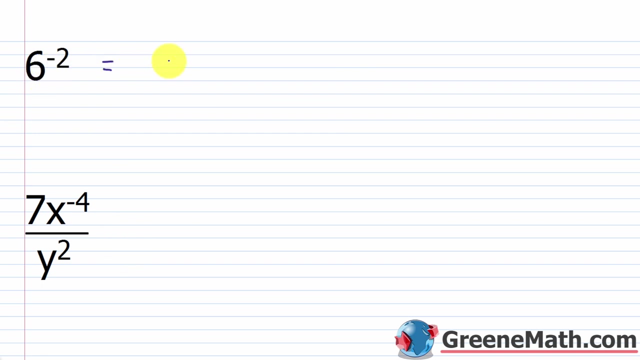 of this, which would be x to the power of m over 1, which equals x to the power of m. So that's how I got that kind of in a longer format, All right. so two quick examples. Let's say, you see, 6 to the power of negative 2. All this is is it's 1 over 6. 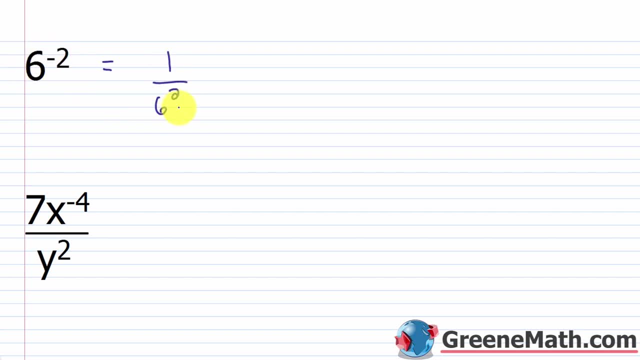 squared. Take the reciprocal of the base. make the exponent positive. The reciprocal of 6 is 1 over 6.. If I make the exponent positive, instead of being negative, 2, it's positive 2.. You could leave it like this: 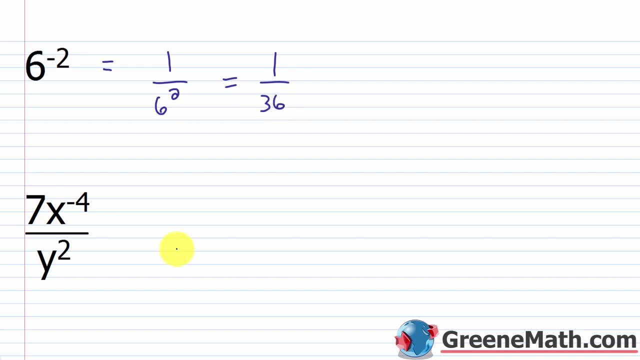 or you can write 1 over 36. And it looks pretty cool again. another way to think about this, or an easier way to get the answer, is just to set up a little fraction bar here and say: okay, I'm going to drag this down here, I know there'll be a one up here. 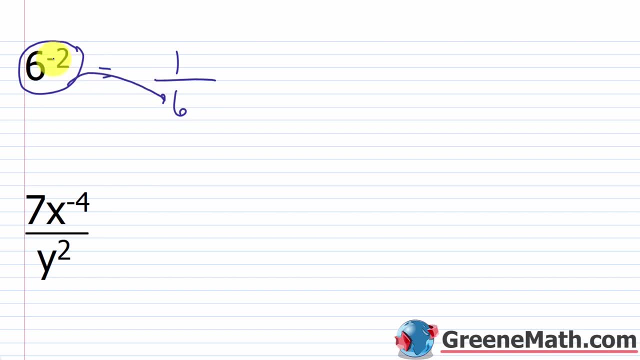 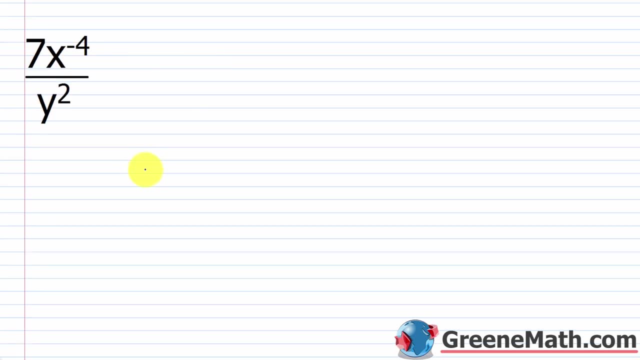 now, and so, if I drag this down here, six will be the same, but the sine of the exponent is going to be positive now, so this would be one over six squared. all right, then for the next example, we have seven times X to the power of negative, 4 over Y squared. so, again with this part, right here. 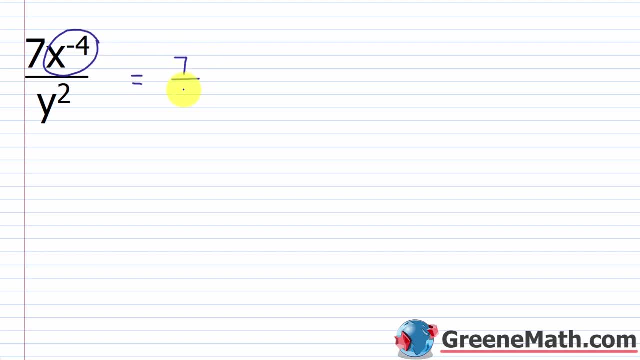 I could separate this and say this is 7 over Y squared, times X to the power of negative 4. you can put it over 1 if you wanted to, it doesn't matter. if I take the reciprocal of this, what would that give me? so it would be 1 over X to the fourth power. so this would be 7 over Y squared. 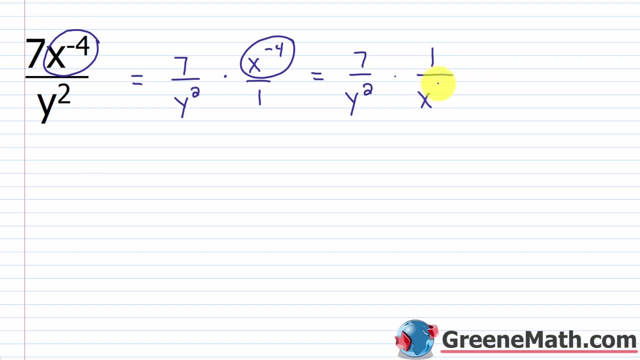 times 1 over X to the fourth power, which, which would be seven over, you'd have y squared times x to the fourth power. Now another way to kind of think about this and what I always do: if I have seven x to the power of negative four. 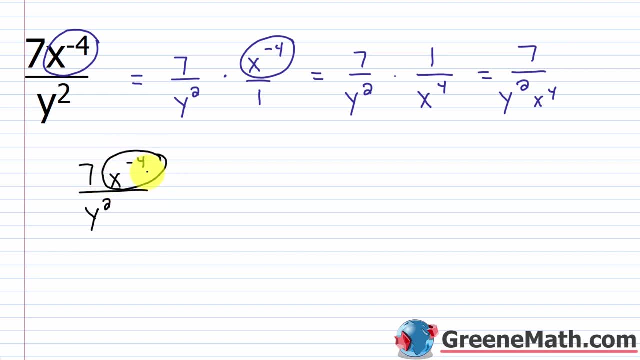 over y squared. you're just going to bring this down here. And again, when I cross the fraction bar, the exponent is going to be positive instead of negative, So I can erase this up here And either way I do it. this is seven over y squared times x to the fourth power. All right. 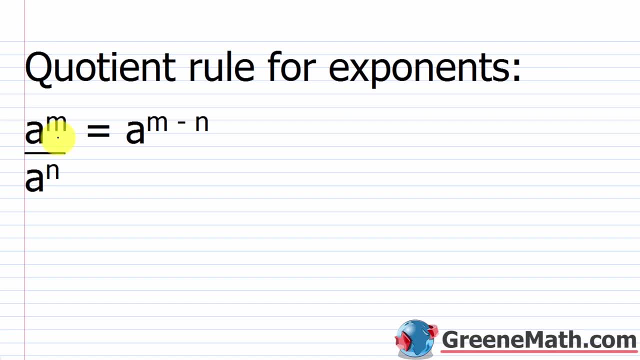 the next rule. let's talk about the quotient rule for exponents. So if we have the same base and division is involved, we keep the base the same and we subtract exponents. So a to the power of m over a to the power of n is equal to a to the power of m minus n. Let's look at a couple. 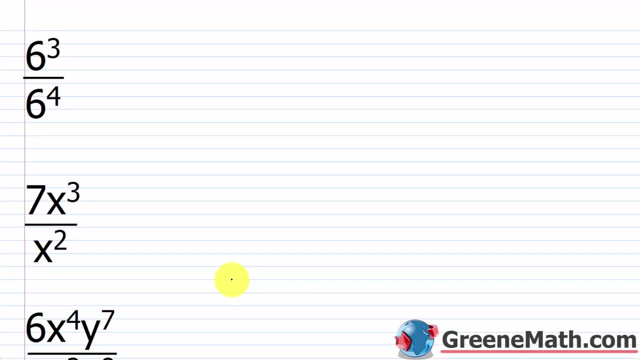 of examples here. All right. for the first example, we have six cubed over six to the fourth power. So we have the same base here of six. So what I'm going to do is keep that base the same and I'm going to subtract the exponent. So I'm going to subtract the exponent. 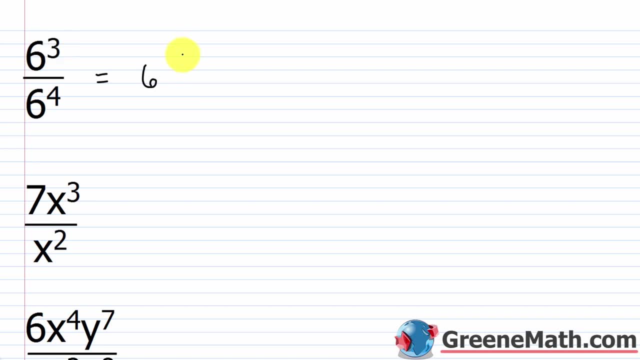 Now, to be more specific, I'm going to take the exponent of the numerator, which is three, and I'm going to subtract away the exponent of the denominator, which is four. Now, three minus four is negative one, So this will give me six to the power of negative one, which we just learned. 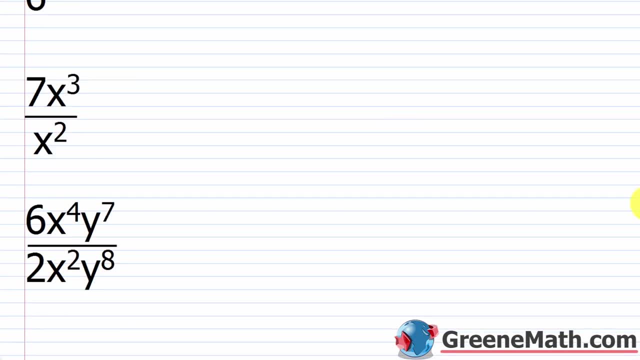 as one over six. All right, for the next one, I have seven x cubed over x squared, So I can write this as seven times x cubed over x squared, And what we can do here again just stays the same. That's unaffected. We have the same base, So x stays the same When we subtract. 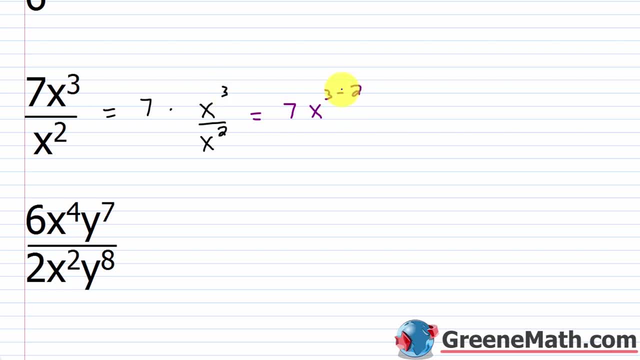 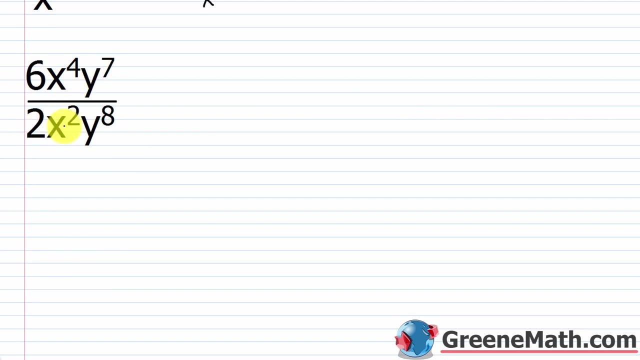 three, the exponent of the numerator, minus two, the exponent of the denominator, and I end up with x to the power of one or just x, So this would be seven x. All right, for the next problem, we have six x to the fourth power, y to the seventh power, over two, x squared, y to the eighth power. 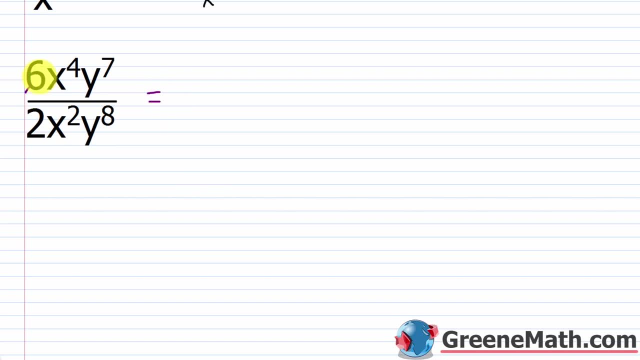 So there's more things I can do here. So I can do this six with this two and get a three. That's how I'm going to start. Then I have x to the fourth power over x squared, So that's x to the power of four minus two. Again, base stays. 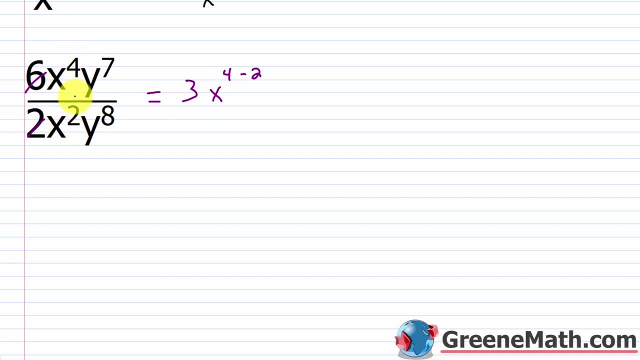 the same, Four is the exponent of the numerator Subtract away the exponent of the denominator, which is two. Then I have y to the power of seven minus eight, Y and y, so y stays the same. The exponent of the numerator is a seven Subtract away eight, which is the exponent of the denominator. 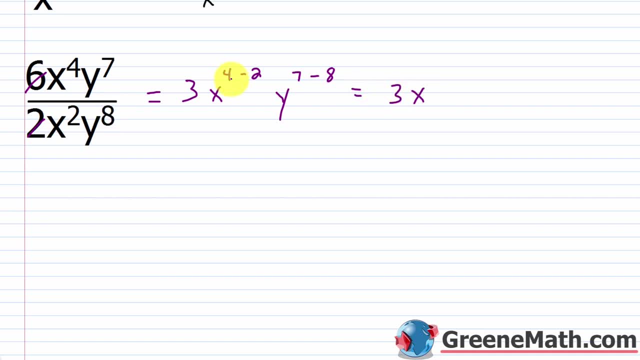 So that's x to the fourth power over x squared. So that's x to the power of four minus two. So this gives me three times x to the power of one. Four minus two is two, So three x squared. then times y to the power of seven minus eight is negative one, So I could rewrite this as three x. 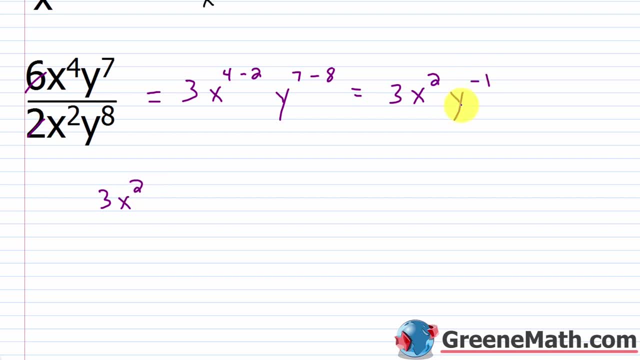 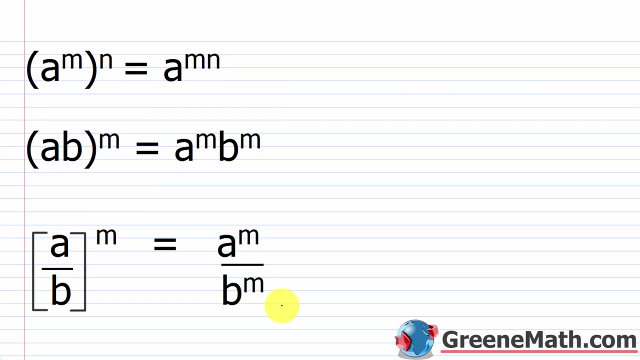 squared. I can drag y to the power of negative one into the denominator and I would have y to the power of one. The y would stay the same, but the exponent will go from negative to positive because it crosses the fraction bar. All right, the next thing we want to think about will be some power rules. 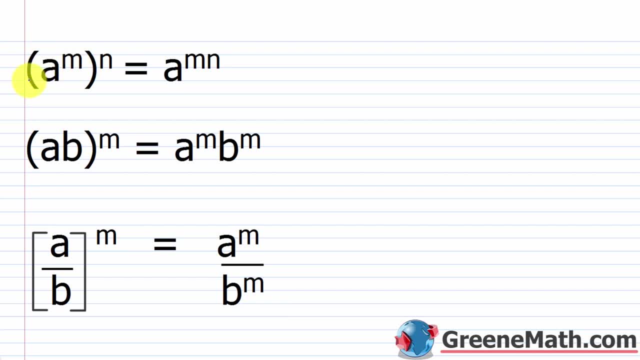 So we see something like a raised to the power of m- This is inside of parentheses- and it's raised to the power of n. This is equal to a to the power of m times n. So in other words, if I have a power already and I raise that to another power, it's called the power to power. 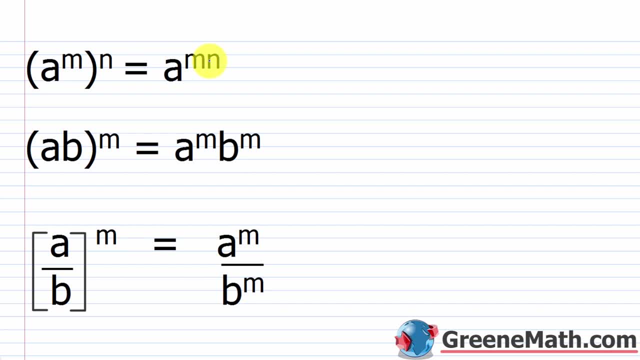 rule, I keep the base the same and I multiply exponents. So if I saw something like two cubed and I squared this, two would stay the same and I'd multiply three times two to give me six. So this would be two to the sixth power. You could prove that to yourself. Two cubed is eight. 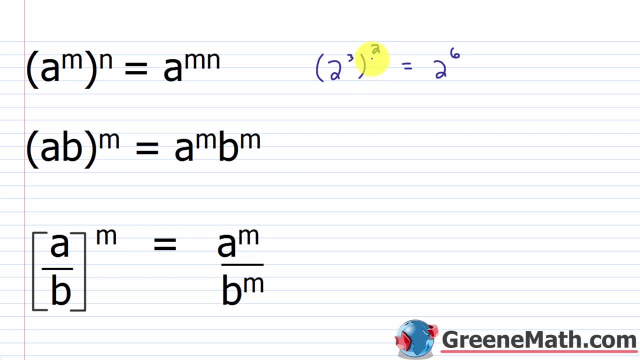 If I had eight and I squared it, I would get 64.. Now, two to the sixth power we know is 64. So either way, you can see, that would be 64.. Now, as the next example, if we had a times b here. 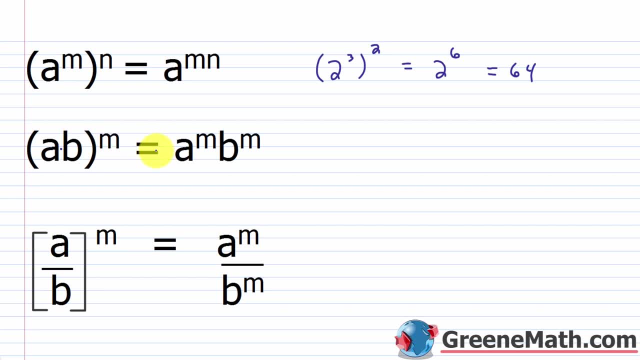 and this whole thing was raised to the power of m. I can say this is equal to a to the power of m times b to the power of m. so as an example of this, let's say we saw 2 times 3 and this was raised to the third power. let's say: 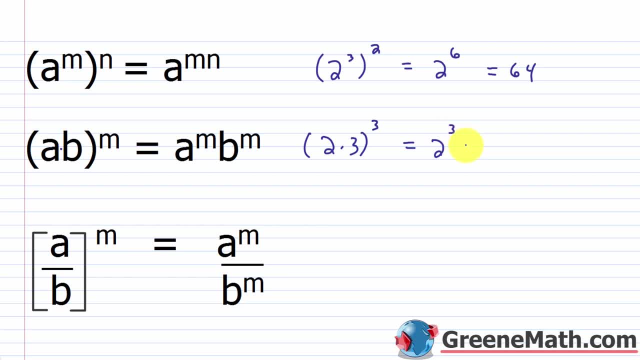 well, I could say: this is 2 cubed times 3 cubed, and you can prove this to yourself as well: 2 times 3 is 6, 6 cubed is 216. if I do it this way, 2 cubed is going to give me 8, 3 cubed is going to give me. 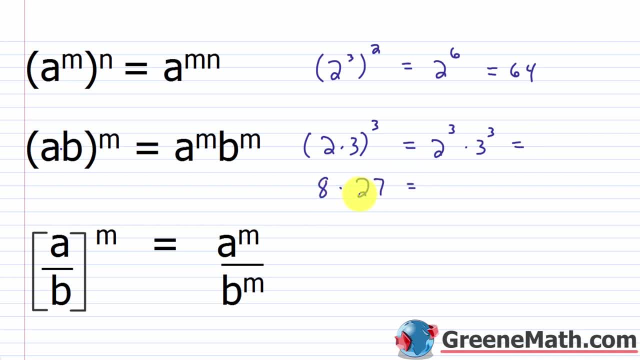 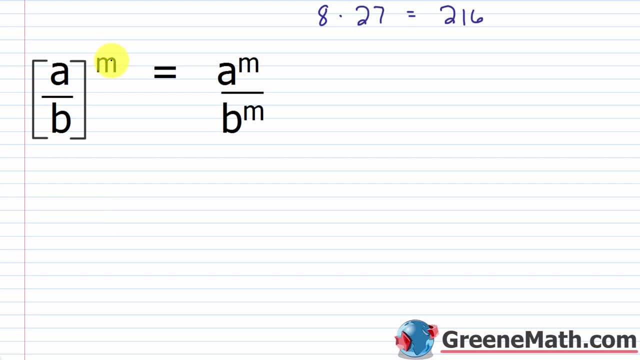 27. if I multiply 8 times 27, I get 216 as well. all right, now we also want to look at: we have a quotient here, a over b. this is raised to the power of m, so we say this is equal to: we have a over m. 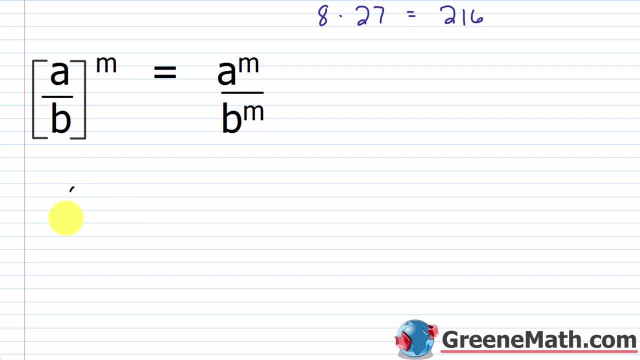 over b over m. so, as an example of this, let's say I had something like 10 over m over 2, and this is squared. Well, this is 10 squared over 2, squared. You can think about this as going here and also here: 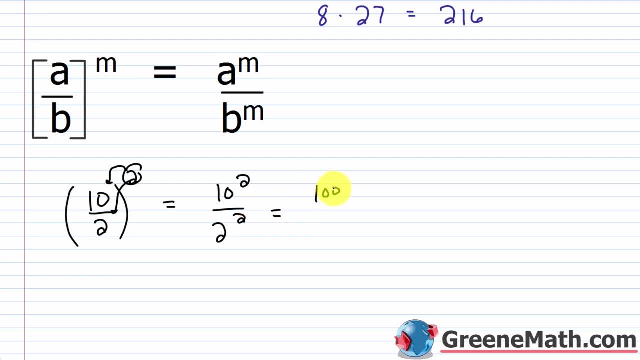 So this would be equal to what 10 squared is 100 over 2 squared, which is 4.. So this is 25.. Now you can think about this another way: 10 over 2 is 5.. 5 squared is 25.. 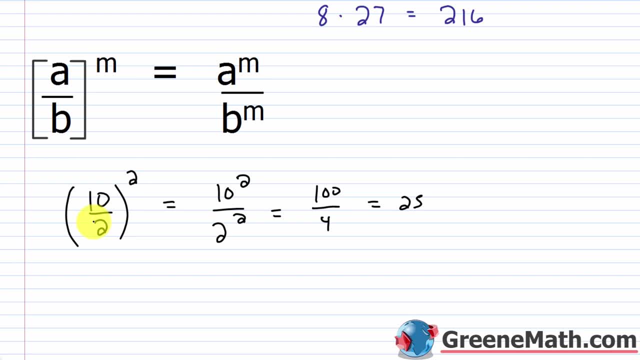 Now you might say: why would you do it this way? It seems like it's quicker with what you just did. Well, it's important to just understand that you can go back and forth. You might see something in this format and say, hey, 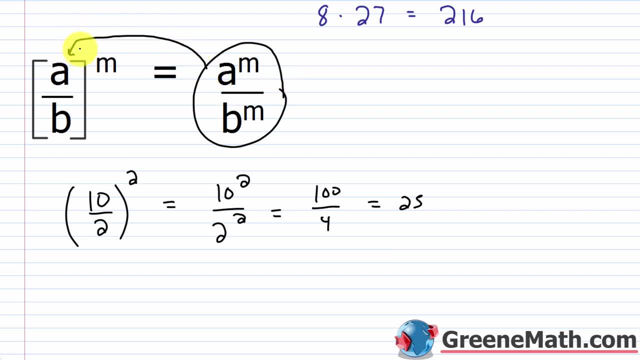 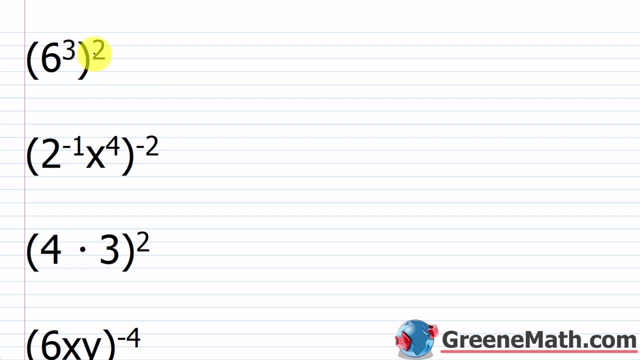 it'd be pretty easy to do that calculation in this format, So you can go back and forth between the two, It doesn't matter, All right. so let's look at some examples. If I have 6 cubed and then it's squared, it's again that power to power rule. 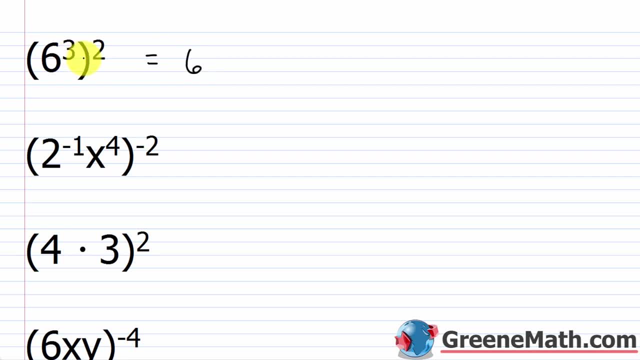 So 6 stays the same and I would multiply exponents 3 times 2 is 6.. So this would be 6 to the sixth power. For this one I have 2 to the power of negative 1.. Times x to the fourth power. 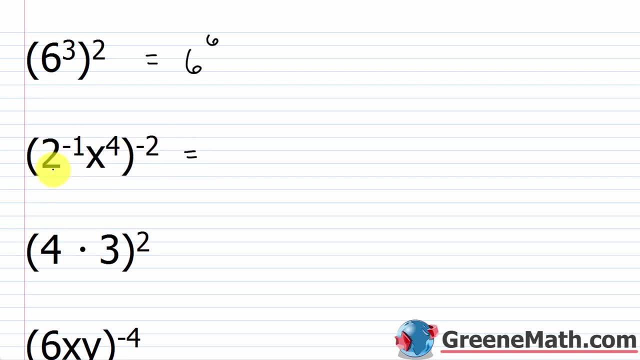 And this whole thing is raised to the power of negative 2.. So again, the base in each case would stay the same. So 2 stays the same And you'd have negative 1 times negative 2, which is 2.. 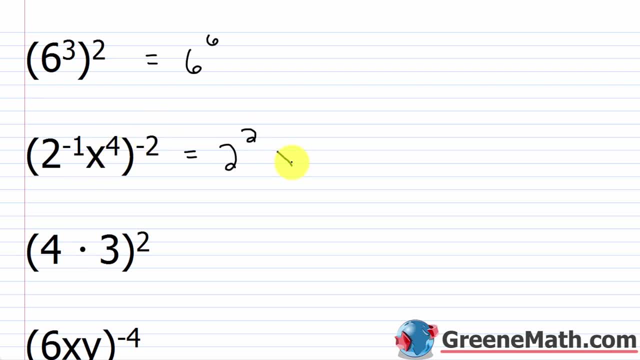 Here I'd have x to the fourth power. So x stays the same And we do 4 times negative 2, which is negative 8.. So the base stays the same and you multiply the exponents. Now, in this case, since we know that x to the power of negative 8. 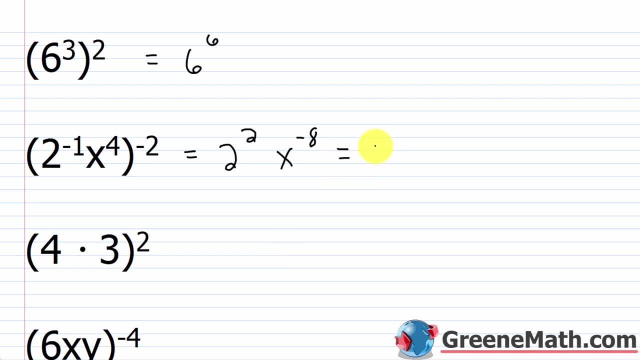 is 1 over x to the eighth power. I can just simply write this as 2 squared over x to the eighth power. Remember, if I grab this right here and I bring it across the fraction line, what I know is x stays the same. 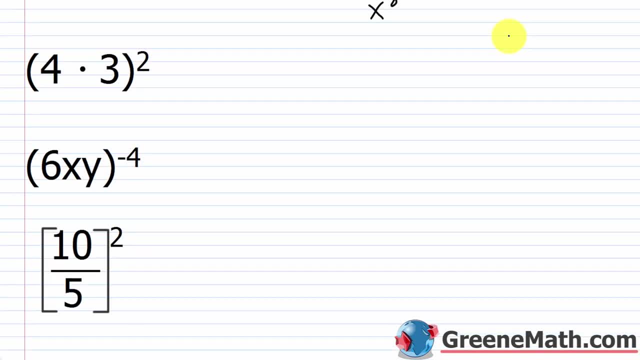 The exponent goes from negative to positive. All right, the next one we're going to look at. we have 4 times 3.. And this is all raised to the power of 2, or you could say it's squared. So this is the same as saying we have 4 squared times 3 squared. 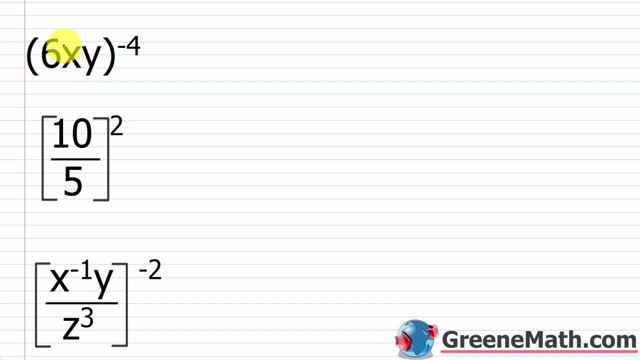 Now let's look at the next one. All right, for the next one, we have 6xy inside of parentheses. This is raised to the power of negative 4.. So I could do this a few different ways. The first way I could do it is I could just take the reciprocal of this guy right here. 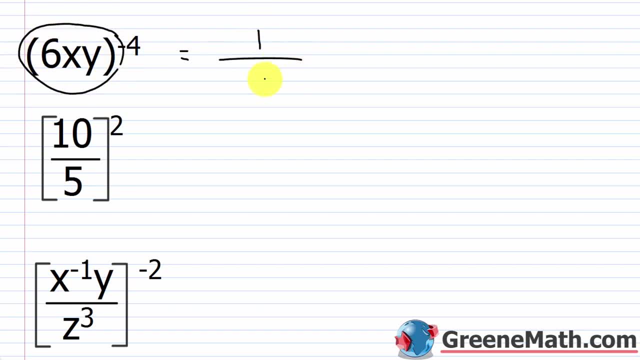 and I could raise it to a positive 4.. So I could say this is 1 over, and then I'll have 6xy- this in parentheses- raised to the power of 4.. Then I would use my power to power rule. 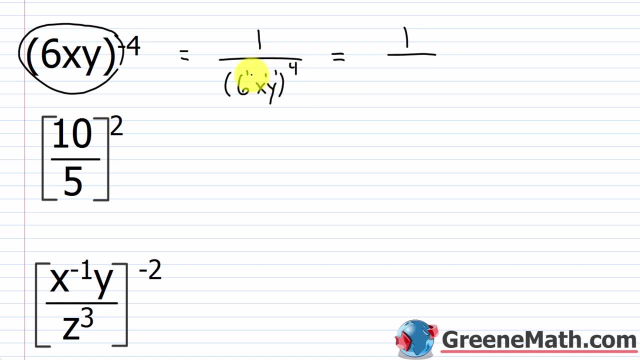 Remember, everything has an exponent of 1 right now. So 4 times 1 would be 4 in each case. So everywhere we'd have 6 to the fourth power, x to the fourth power, y to the fourth power, So everything would have an exponent of 4.. 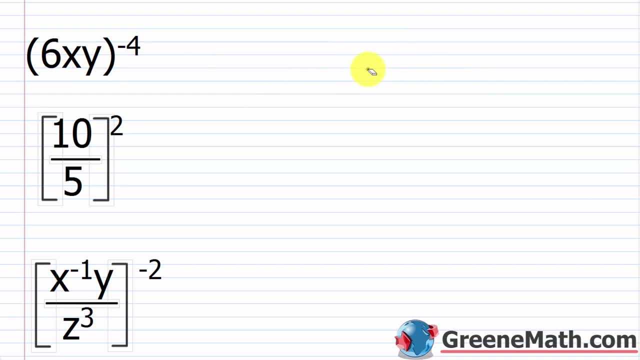 Now another way you could have thought about that. let's just erase this real quick. We could say OK. every exponent here is a 1 inside the parentheses, So I'm just going to say OK. 6 to the power of 1 is raised to the power of negative 4.. 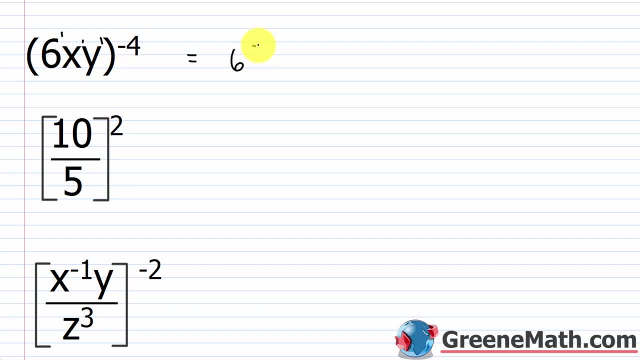 So that would be 1 times negative 4, or negative 4.. So I'd have 6 to the power of negative 4.. Same thing for x. I'd have x to the power of negative 4.. Same thing for y. 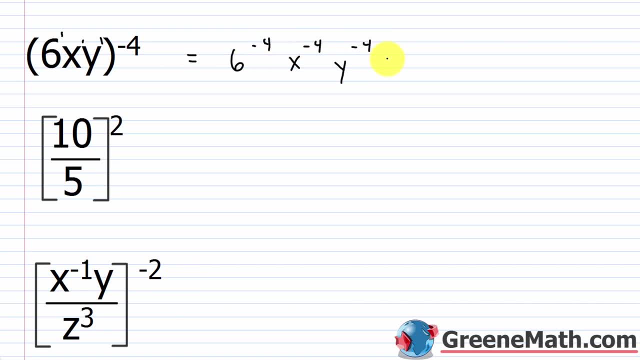 I'd have y to the power of negative 4.. Then, because these are all negative exponents, I can drag everything across the fraction bar, make the exponents positive. So I can have 6 to the power of positive 4, x to the power of positive 4, then y to the. 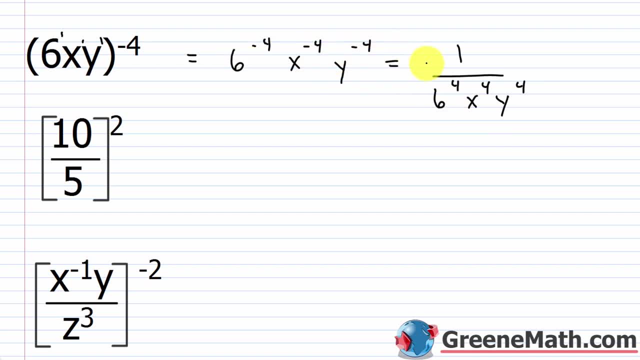 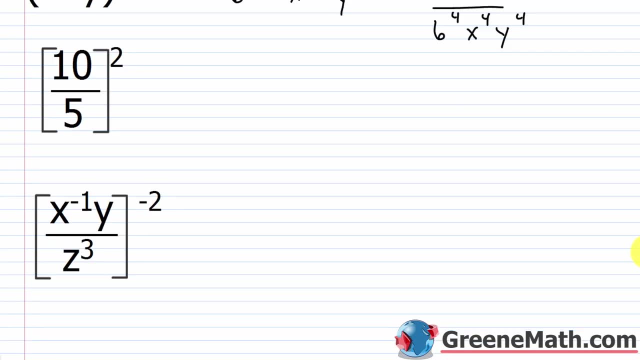 power of positive 4.. Again, I move these from the numerator to the denominator, So I have 1 over 6 to the fourth power, x to the fourth power, y to the fourth power. What about this one? We have 10 over 5.. 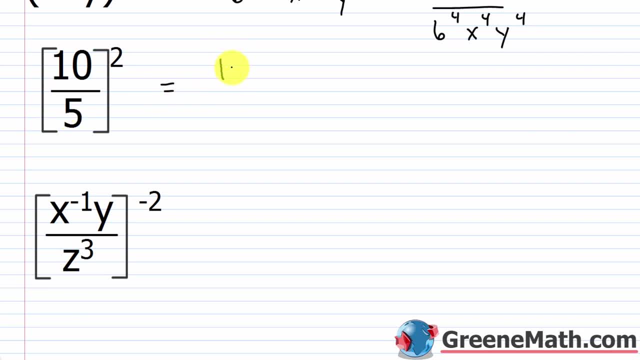 And this amount is squared, So I can write this as 10 squared over 5 squared. And again you can prove that to yourself pretty easily: 10 squared is 100, 5 squared is 25.. The result of this would be 100 over 25, which is 4.. 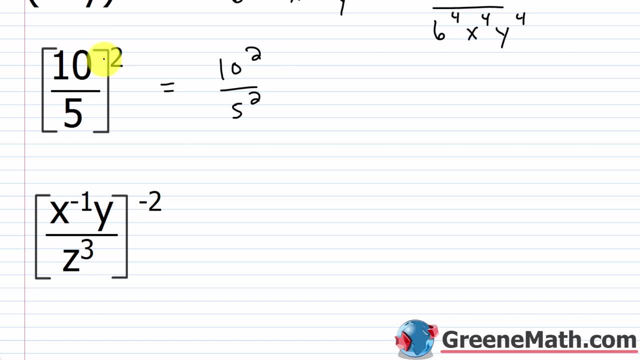 If I did it in here, 10 divided by 5 would be 2., And if I square 2, I get 4.. So either way it's the same, All right. So this is the power of negative 1 times y. 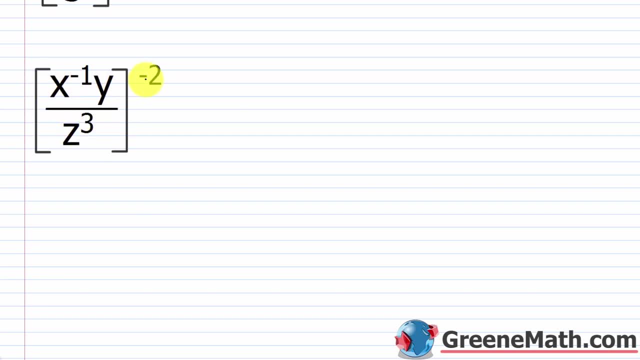 This is over z cubed And then this is inside of brackets and it's raised to the power of negative 2.. So you can think about each base here as staying the same and just multiplying the exponents. So x stays the same. 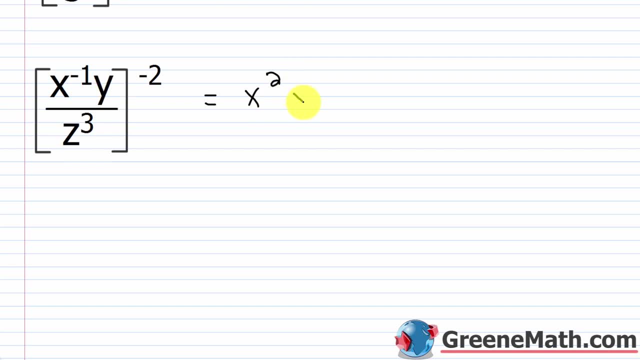 Negative. 1 times negative 2 is 2.. Y stays the same. Remember it has an understood exponent of 1.. So 1 times negative 2 would be negative, 2.. This is over. We have z, which stays the same. 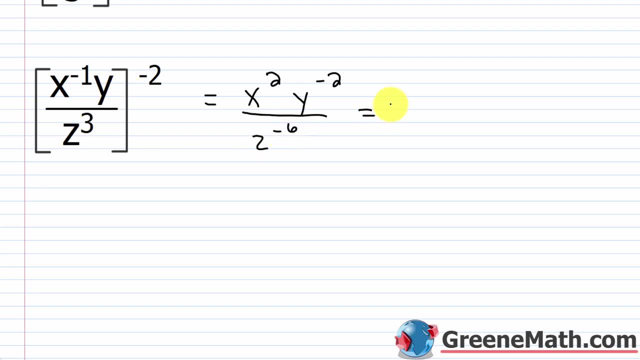 3 times negative. 2 is 2.. This is negative 6.. So now all I want to do- x squared- would stay the same. This would go into the denominator, And so I would change the sign of the exponent So it would be y squared. 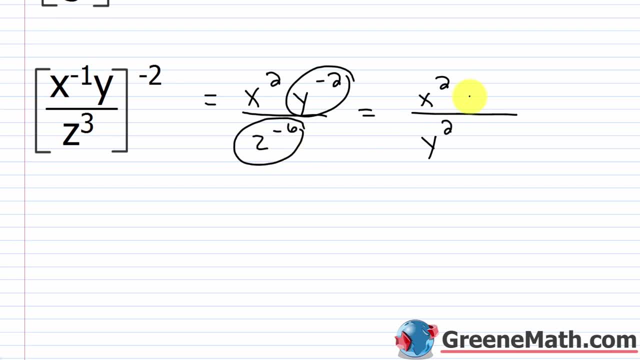 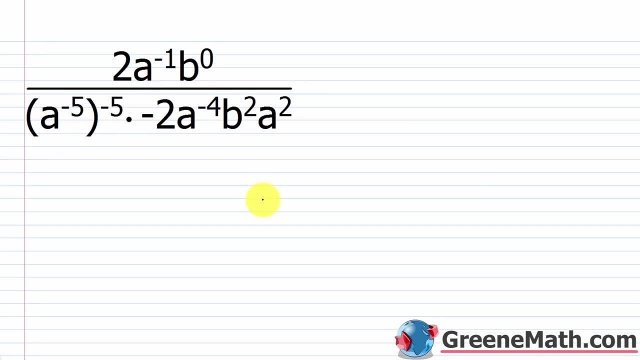 This would go into the numerator, So I'd change the sign of the exponent. It would be z to the sixth power, So x squared times z to the sixth power over y squared. All right, So let's look at a few practice problems before we kind of move on to our topic of polynomials. 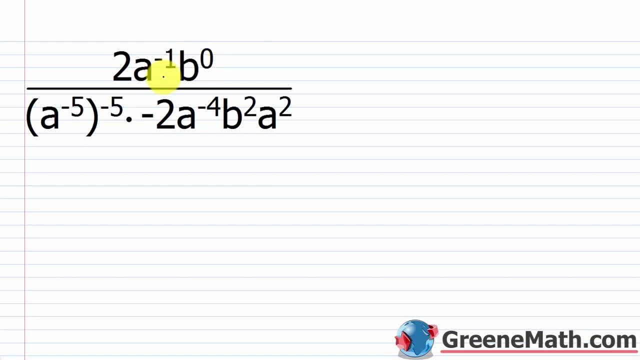 So we have 2a to the power of negative 2.. We have 2a to the power of negative 1 times b to the power of 0. And this is over. We have a to the power of negative 5.. 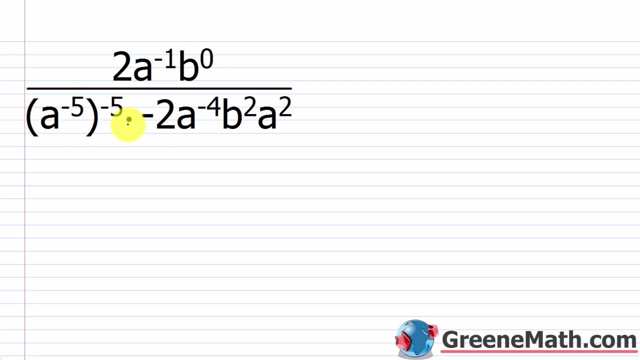 And this is raised to the power of negative 5 times negative, 2a. to the power of negative 4 times b squared times a squared. So if I simplify in the numerator first, I know b to the power of 0 is 1.. 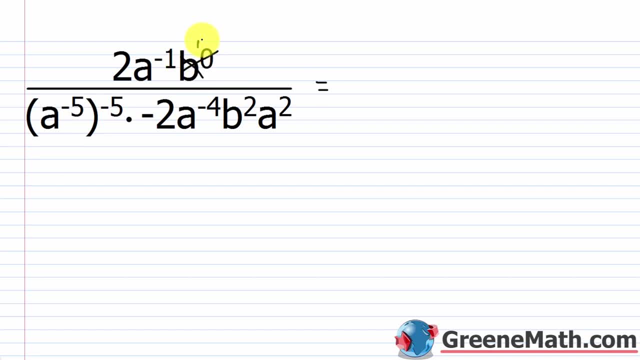 So I can kind of cross this out and just put a 1 there. One times anything is just itself. So the numerator I'm going to write is 2a to the power of negative 1.. So I'm going to put a 1 there. 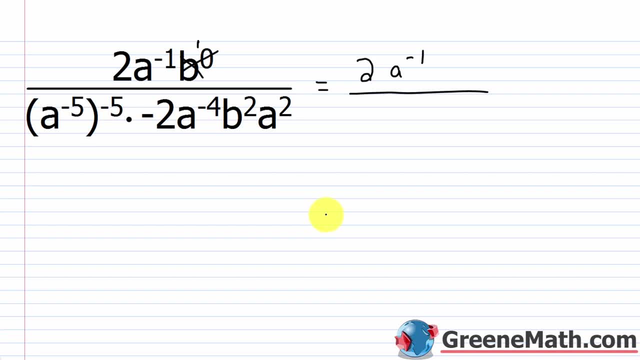 1 times anything is just itself For my denominator. I've got a lot of stuff going on, So I've got a to the power of negative 5 raised to the power of negative 5.. So a stays the same. negative 5 times negative 5 is 25.. 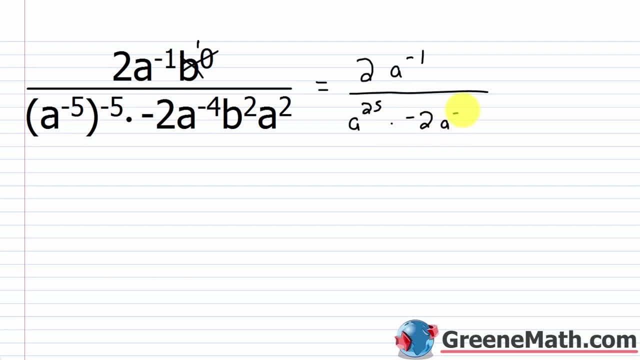 Then times you have a negative 2, a to the power of negative 4, b squared, a squared. So let me write 2a to the power of negative 1 over. I have a to the power of 25, I have. 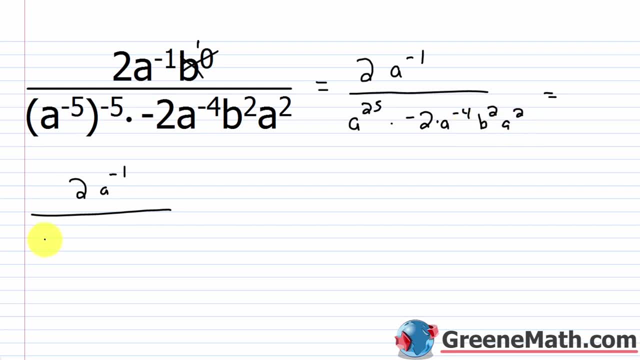 a to the power of negative 4, and I have a squared. So keep a the same and just add those exponents: 25 plus negative 4 is 21,. 21 plus 2 is 23.. So I'll have a to the power of 23 there and I have that negative 2.. 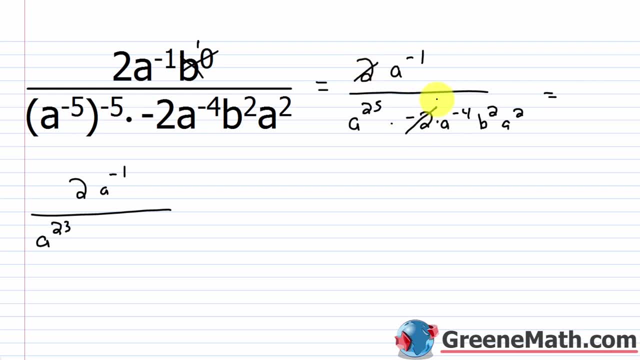 Now what I can do is I can cancel this 2 with a negative 2, and I can put a negative 1 there. So instead of having a 2 there, let me just put a negative in front of that. a to the power. 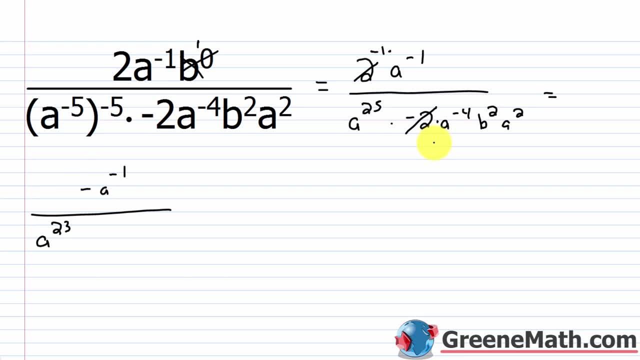 of negative 1.. All right, so now the next thing I have is a b squared. Nothing I can really do with that, so I'll just rewrite b squared. So the last thing is: let me write equals. I'm going to put a negative 1 times I have. 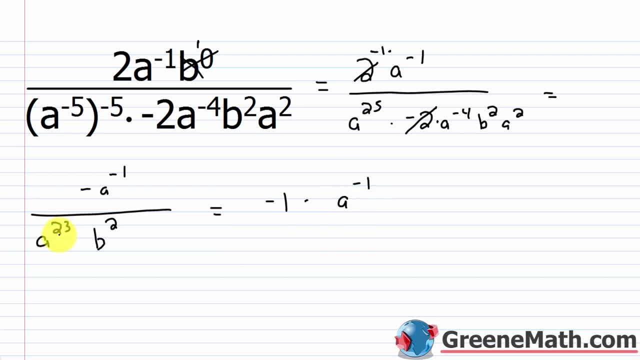 a to the power of negative 1,. now I have an a to the power of 23 here, So what I can do is keep a the same. I would subtract negative 1 minus we have 23 in the denominator. We'd have a to the power of negative 1 minus 23,, which would be negative 24.. 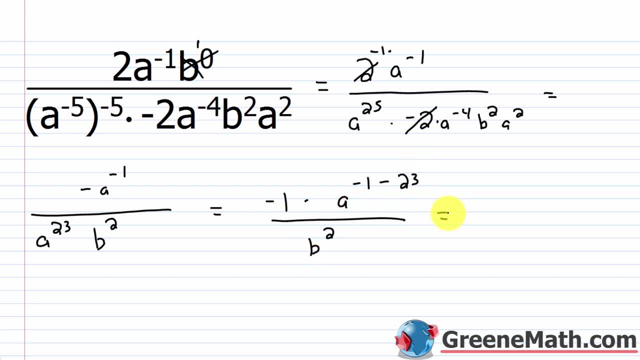 And this would be over b squared. So again, I'll have negative 1 times. we'd have a to the power of negative 1 minus 23,, which would be negative 24. This is over b squared. The last thing I'm going to do is I'm going to put this in the denominator. 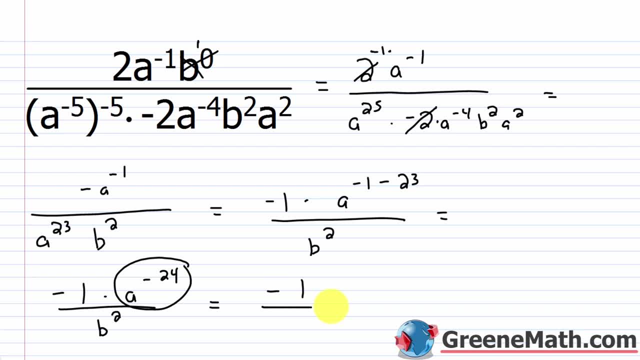 And when I do that I'll have negative 1 over b squared times this. a will be the same but the exponent- because I'm dragging it into the denominator- will be positive. So a to the power of 24.. So negative 1 over b squared times a to the power. 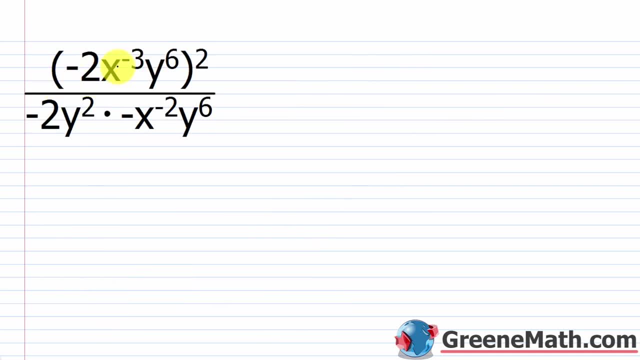 of 24.. All right, for the next one, we have negative 2x to the power of negative 3, y to the power of 6.. This is inside of parentheses and it's all squared. Then this is over, We have. 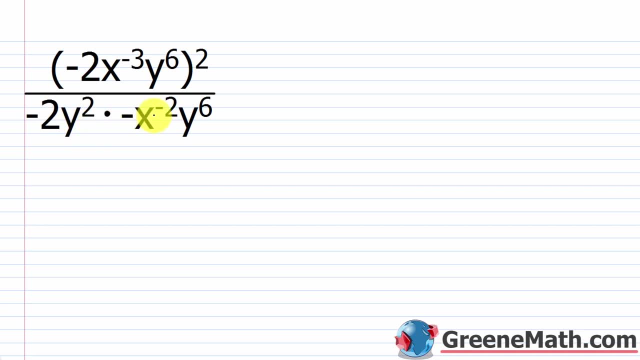 negative 2y squared times negative x to the power of negative 2 times y to the sixth power. So let me start out in the numerator here. Just think about this is going to be applied to everything. All right, that's your power to power rule. Now I want you to be very, very careful here. 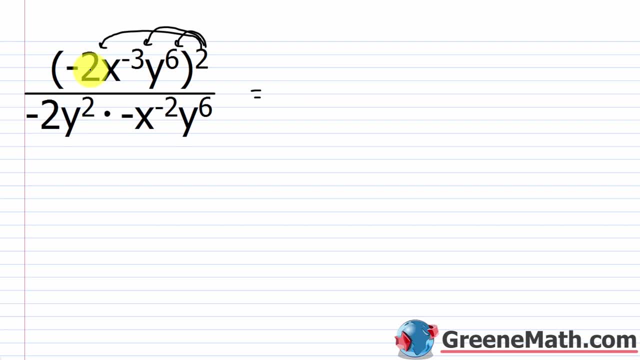 This negative 2 is inside of parentheses. It's inside of these parentheses here, So that negative and that 2 are both squared. So I could do this two ways. I could say I have negative 2 like this squared, or I could treat this negative as. 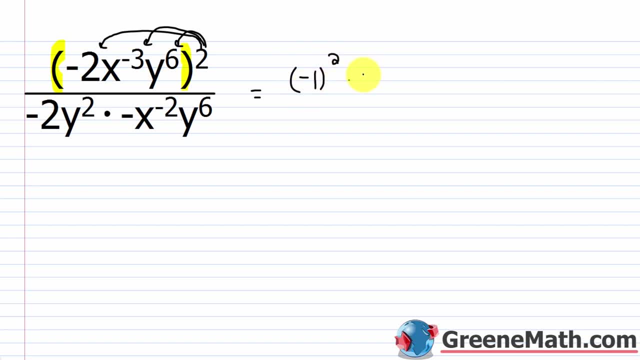 a negative 1 and say that's squared, then times 2 squared, then times x to the power of negative 3 squared, then times y to the sixth power squared, And if I go through on each thing, negative 1 squared is 1.. So this is 1. 2 squared. I'm just going to leave it like that for now. 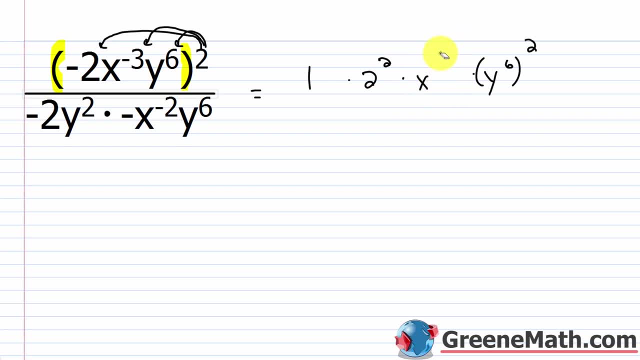 x to the power of negative 3, squared would be x to the power of negative 6.. And then y to the sixth power raised to the second power. of y to the sixth power, squared would be y to the 12th power. Then this is over. I have a negative 2, which I'm going to write as negative 1 times 2.. 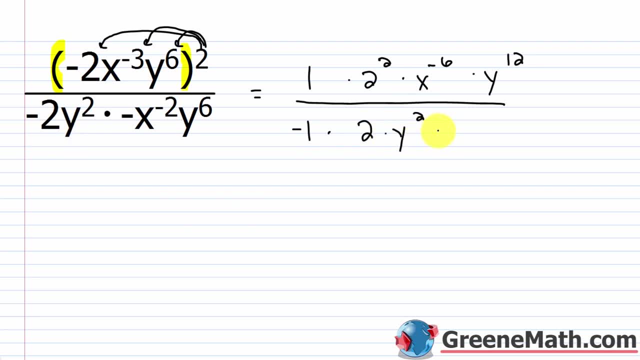 Then I have y squared, Then I have a negative x. So I'm going to write negative 1 times x. This is raised to the power of negative 2, then times y to the sixth power. So a lot of things we can do. 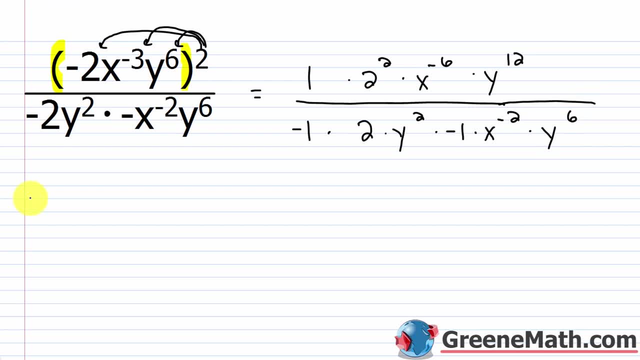 And I want to go slowly. I know a lot of you can do this much quicker, but I want to go slowly so everybody can follow along. So let me just start by simplifying in the denominator real quick. So in the numerator I'm going to leave this as 2 squared times x to the power of negative 6. 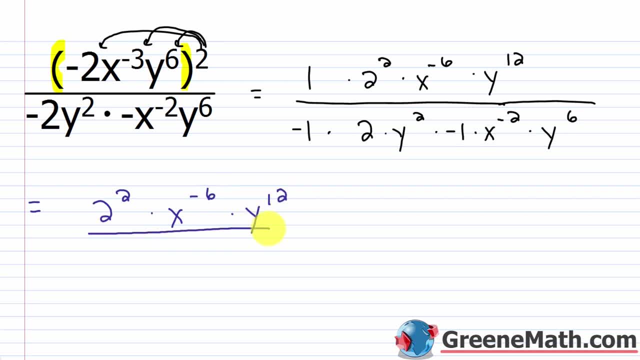 times y to the 12th power In the denominator I'm going to leave negative 1 times 2.. What I'm going to do is I'm going to say I have y squared times y to the sixth power. y stays the same: 2 plus 6 is 8.. Then I have times another negative 1.. 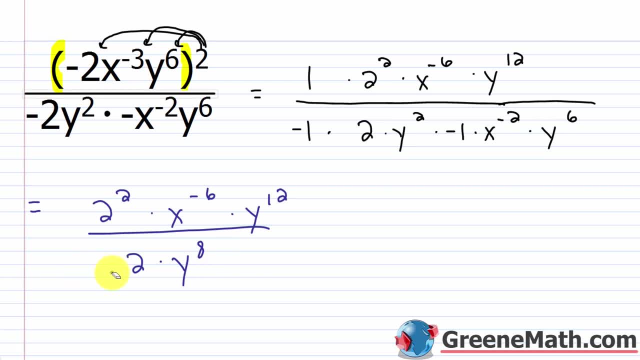 So negative 1 times negative 1 is 1.. So we can erase both of these, okay, And I'll just slide this down, And the next thing I see is times x to the power of negative 2.. So what I know is, if I have the same base here, I have 2 squared and I have 2 down here. 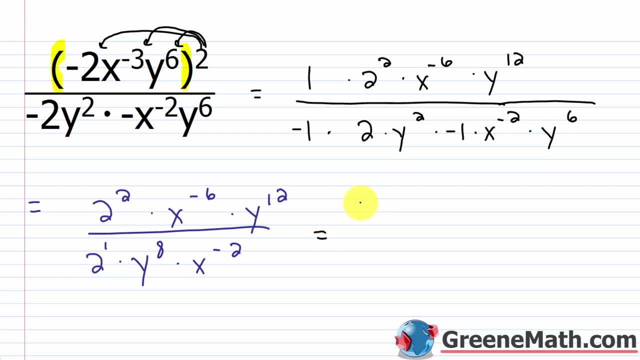 You think about this as 2 to the first power. This is going to tell me I have 2 to the power of what Subtract exponents You'd have 2 minus 1 or 2 to the power of 1.. 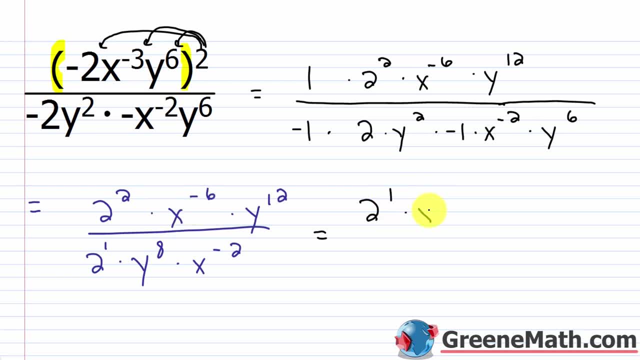 Then next I have x to the power of negative 6. And I'd subtract away a negative 2 because I have x to the power of negative 2 down here. Again, this seems a little weird, but if I have a negative 6 here, that's what I start out with. 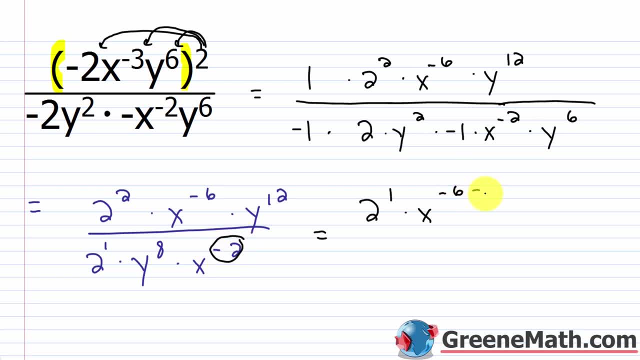 I'm subtracting away a negative 2. Minus a negative is plus a positive. So negative 6 plus 2.. So negative 6 plus 2 is negative 4.. So this would be x to the power of negative 4.. 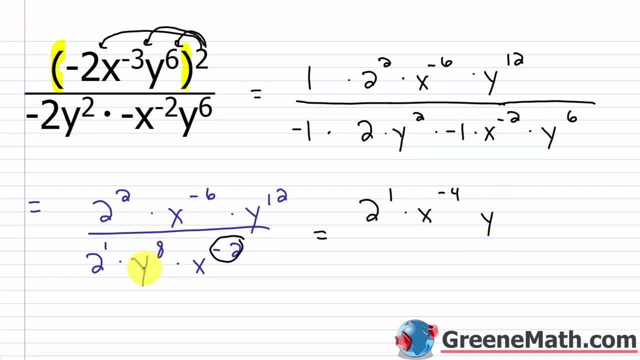 Then, lastly, I have y to the power of 12 here, y to the power of 8 here. So this would be y to the power of 12 minus 8, or y to the fourth power. So if I wrote this over 1, I could drag this down here and say: this is what. 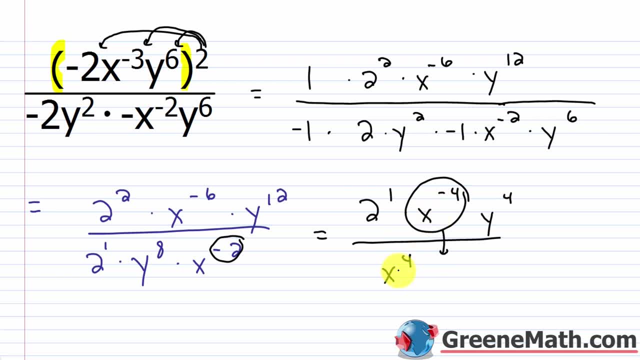 This is x to the power of 4.. x stays the same. The exponent's sign is going to change, So I can just erase. Erase this and say we have 2y to the fourth power over x to the fourth power. 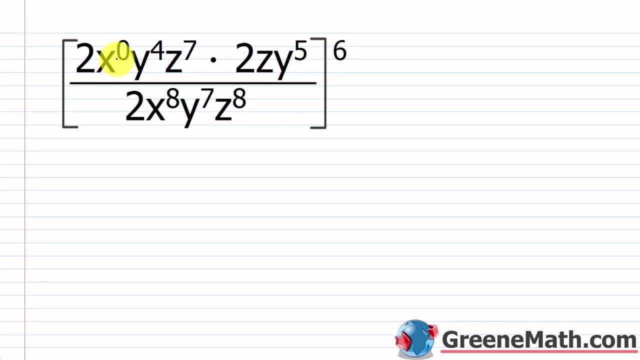 All right. So for the last example, we have 2x to the power of 0,. y to the fourth, z to the seventh times, 2zy to the fifth, over 2x to the eighth power. y to the seventh, z to the eighth. 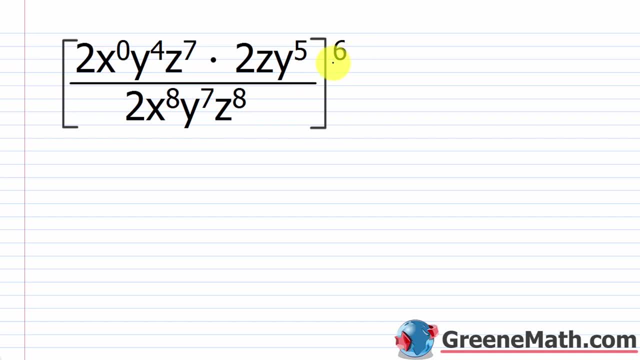 Everything's inside of brackets and raised to the sixth power. So that means that every item inside here is raised to the sixth power. So 2 is raised, It's the sixth power. x to the power of 0 is raised to the sixth power. 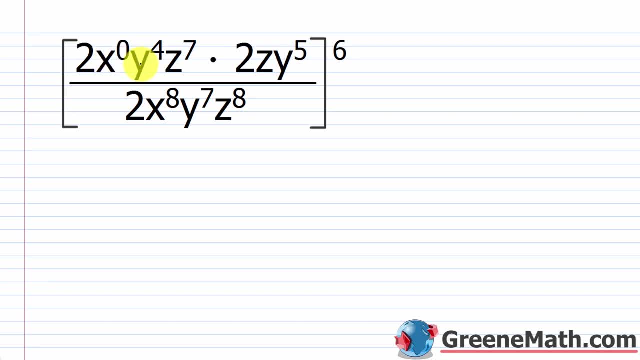 y to the fourth, is raised to the sixth power, So on and so forth. Now you could go through and do that now, but it's going to be easier if you simplify what's inside the brackets first. So let's do that and let's do it in a quick manner. 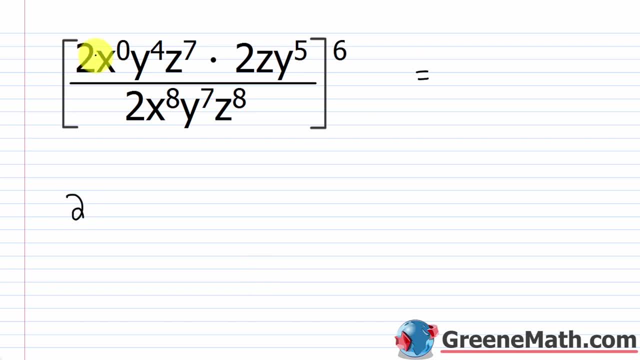 So I'm going to start out with 2.. I have a 2 here and a 2 here, So same base. I would add the exponents. So this is a 1 and a 1.. Right, The exponents are understood. 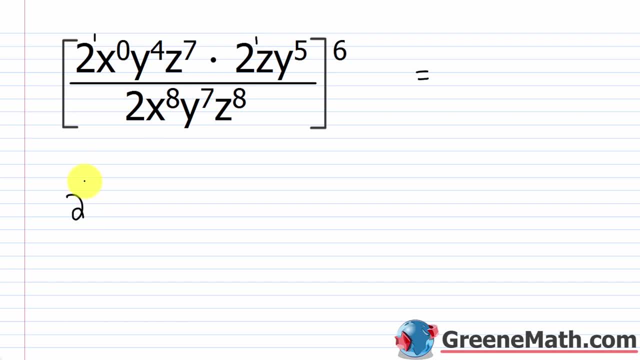 It would be 1 there. So that would be 2 to the power of 1 plus 1, which is 2 squared. Now I also have a 2 in the denominator, So if I had 2 squared over 2, the exponent down here is a 1 as well. 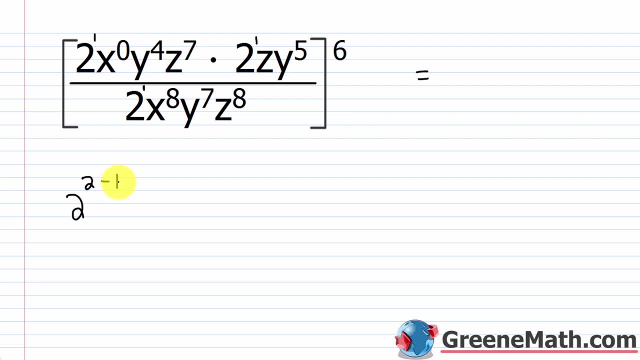 That would be 2 to the power of 2 minus 1.. And so this would be 2 to the power of 1.. The next thing I come across is x. So here I have x to the power of 0, which is 1.. 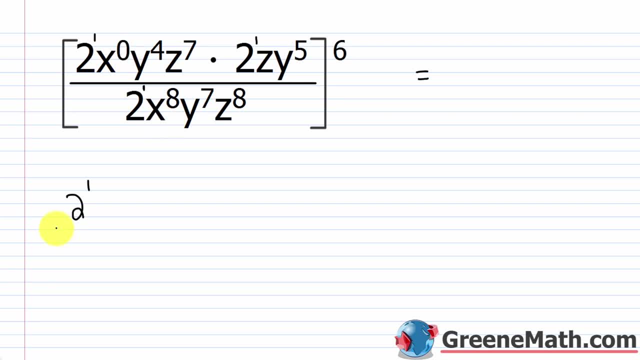 And down here I have x to the power of 8.. So I'm just going to leave that x. I'm just going to leave that x to the power of 8 down there. Then next I come across a y. So y to the fourth power. 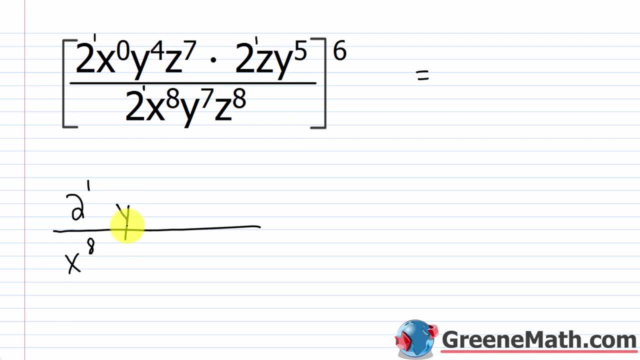 I have a y to the fifth power here. So again, if I did my product rule for exponents y stays the same. I'd add 4 plus 5. That would give me 9.. But then I have a y to the seventh power of the denominator. 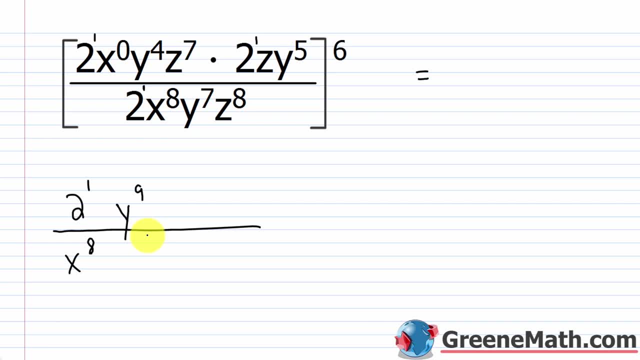 So for that use, the quotient rule for exponents y stays the same. I would do 9 minus 7, which would give me 2.. And then the next thing I come across is z. So I have z to the seventh power here. 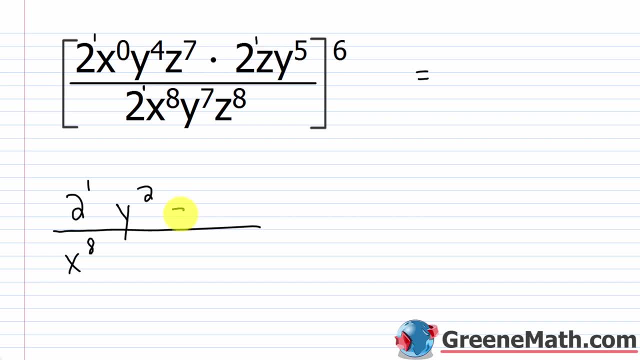 I have a z here. So the product rule for exponents tells me that z stays the same. 7 plus 1 would be 8.. Then down here I have z to the eighth power. So what would happen is I would have z to the eighth power over z to the eighth power. 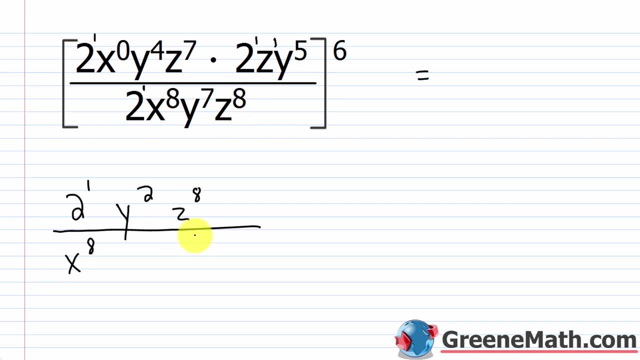 which is 1,. right, Or you can think about it this way: I would take the exponent in the numerator, which is 8,, subtract away the exponent in the denominator for z, which is 8.. That would be z to the power of 0,, which is 1.. 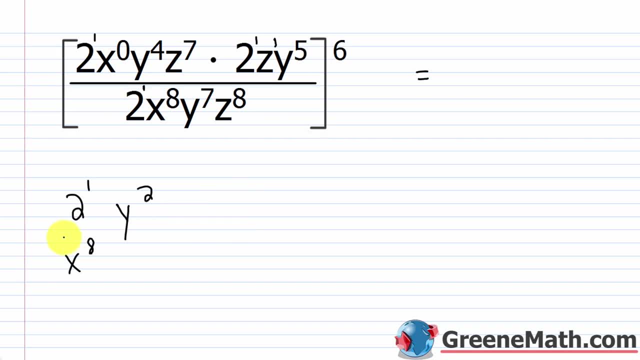 You can get rid of z, All right. so we've dealt with all of that. So don't forget your brackets here. And this is all raised to the sixth power. So 2 to the first power is raised to the sixth power. 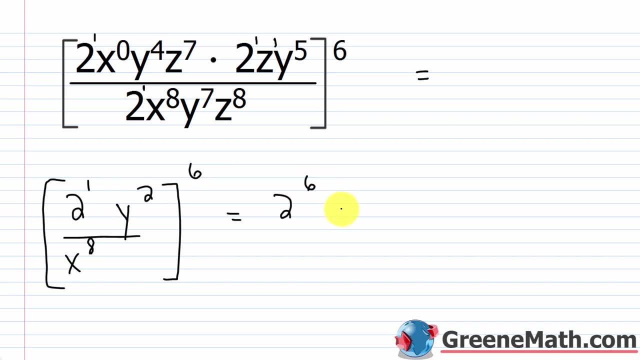 2 stays the same. Multiply 1 times 6, you get 6.. y, squared, is raised to the sixth power. y stays the same. 2 times 6 is 12.. So that's y to the 12th over. 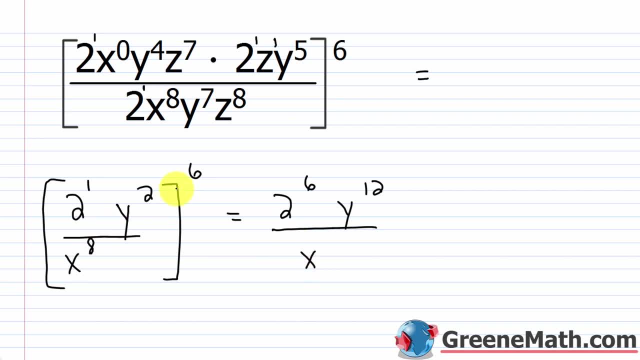 x to the eighth is raised to the sixth power, x stays the same. 8 times 6 is 48. So we get 2 to the sixth power, times y to the 12th power over x to the 48th power. 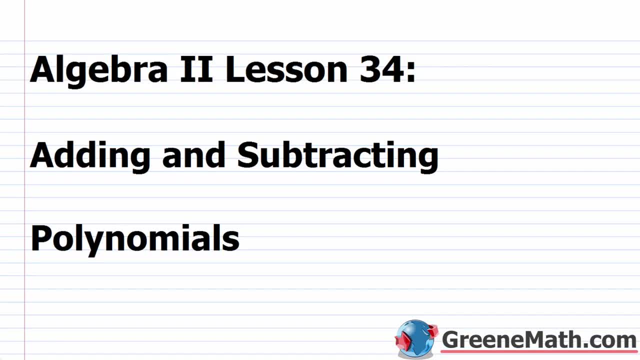 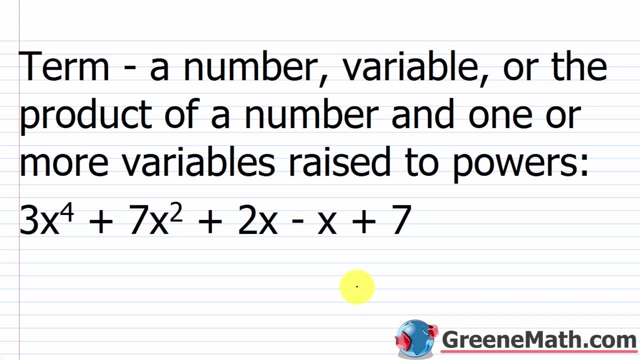 Hello and welcome to Algebra 2, Lesson 34.. In this video we're going to learn about adding and subtracting polynomials, So at this point we should all know the basic definition of a term. So a term is nothing more than a number, a variable. 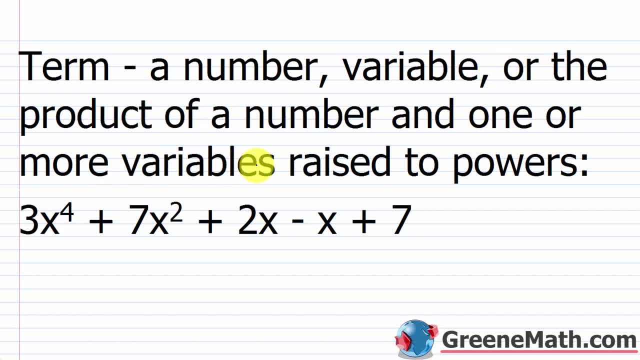 a product of a number and one or more variables raised to powers. So here, to give an example of a term, I have the term 3x to the fourth power plus the term 7x squared plus the term 2x minus the term x. 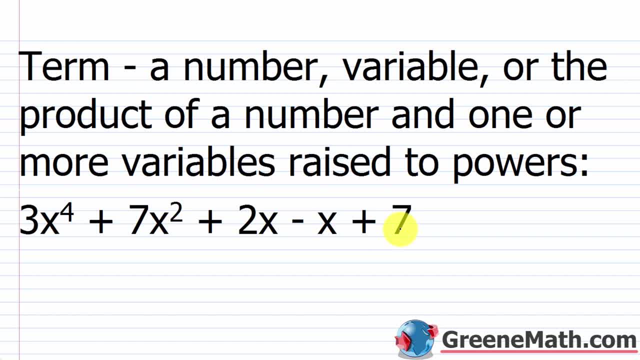 and then plus the term 7.. Now we separate terms with plus or minus symbols. So in other words, everywhere I see a plus or a minus, I'm subtracting, I'm separating my terms. So this 3x to the fourth power is a term. 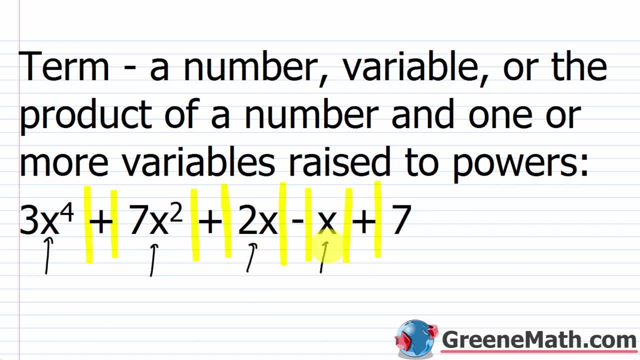 7x squared is a term, 2x is a term, x is a term and 7 is a term And if you go through those individually they fit the criteria given in this definition. We have a number, so a single number like 7,. 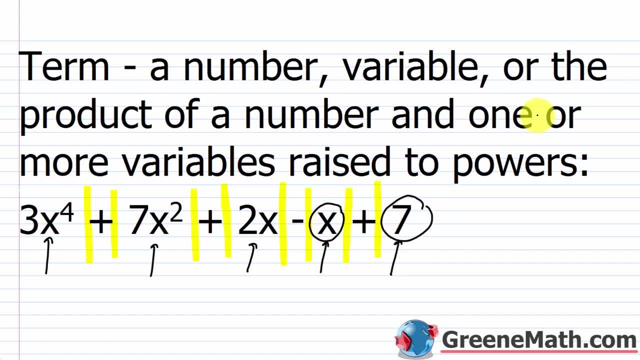 a variable, so just a variable like x or the product of a number, and one or more variables raised to powers. So I have 2 times the variable x, I have 7 times the variable x that's squared and I have 3 times the variable x that's raised to the fourth power. 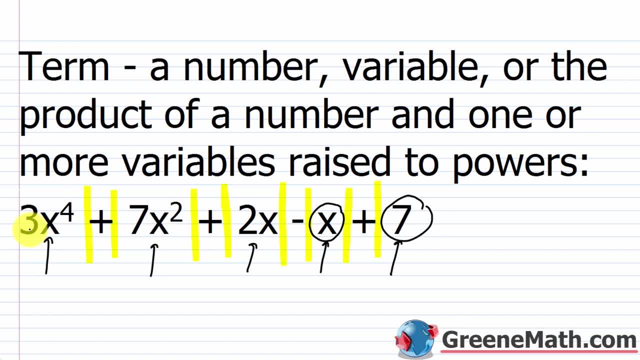 So each of these here again. so 3x to the fourth power, 7x squared, 2x, x and 7, those are all examples of a term. All right, so next let's give a definition for a polynomial. 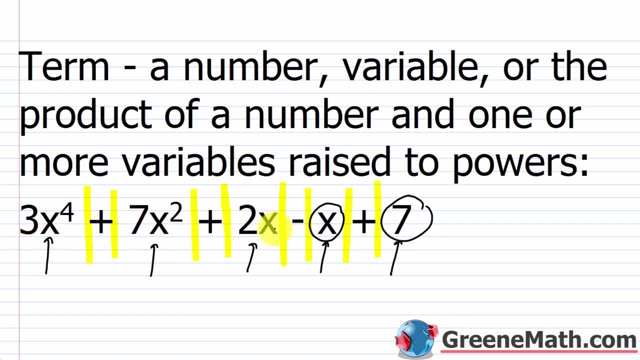 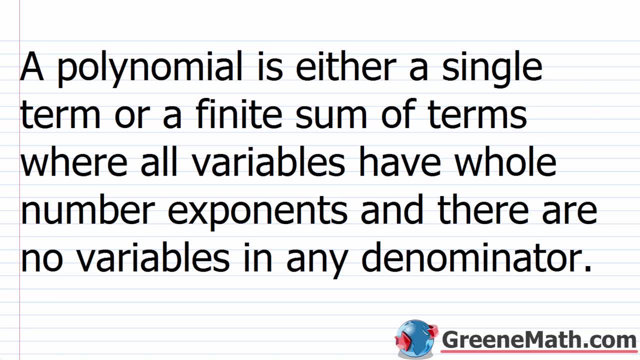 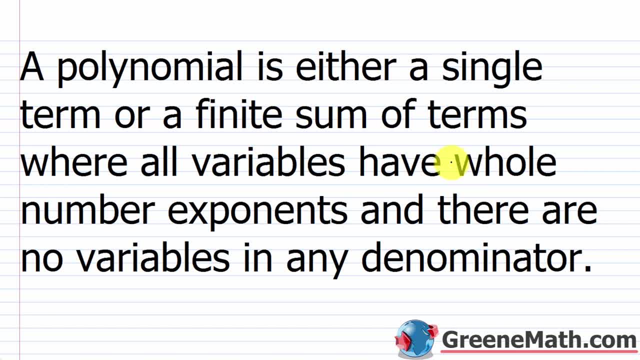 or a finite sum of terms, where all variables have whole number exponents. so we know what a whole number is: that starts with zero and increases in increments of one, forever and ever and ever. and there are no variables. let me highlight this: there are no variables. 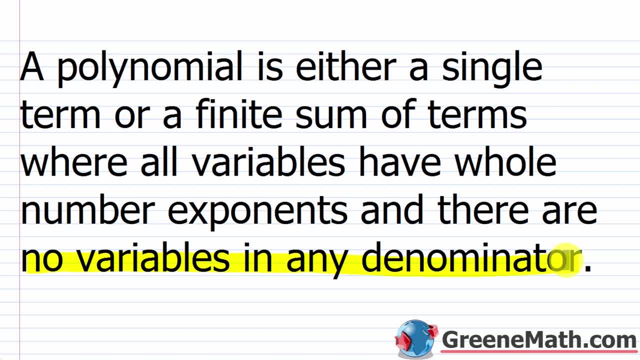 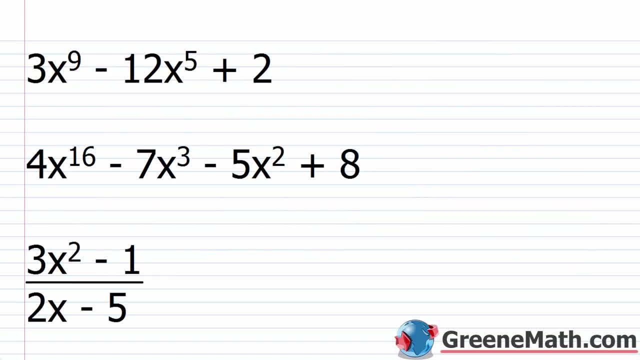 in any denominator. So you want to look out for two things: Whole number exponents and no variables in any denominator. So that's what's going to trip you up. So I'm going to give you two examples of a polynomial. So 3x to the 9th, power minus. 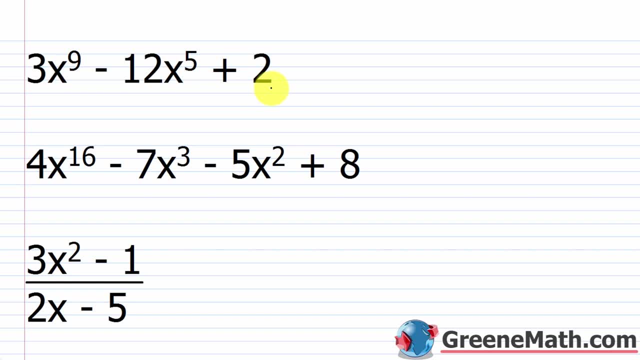 12x to the 5th power plus 2.. This is a polynomial And all you're looking for is, on every term, do I have a variable where we don't have a whole number as the exponent or where we have a variable in the denominator? 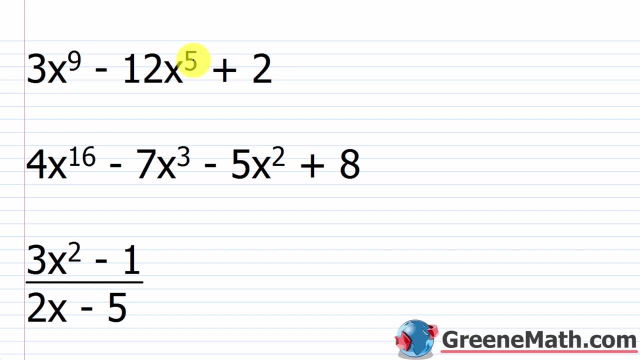 If I look here, I have x to the 9th power and I have x to the 5th power. there's no variable in any denominator. so this is a polynomial. So we're good to go there. Here's another example of a polynomial. 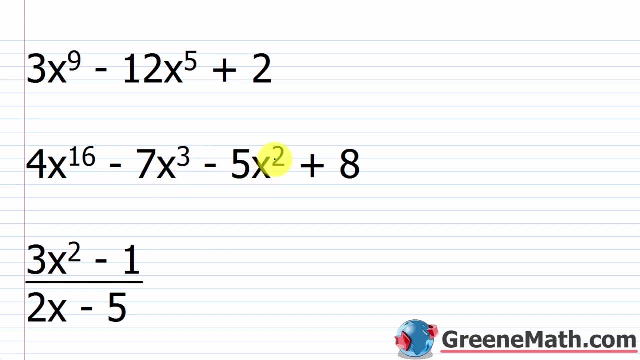 We have 4x to the 16th power, minus 7x cubed, minus 5x squared plus 8.. So I look at my exponents. here I've got a 16,, a 3, and a 2.. 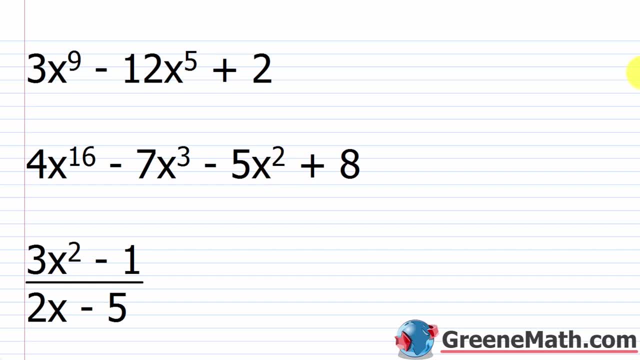 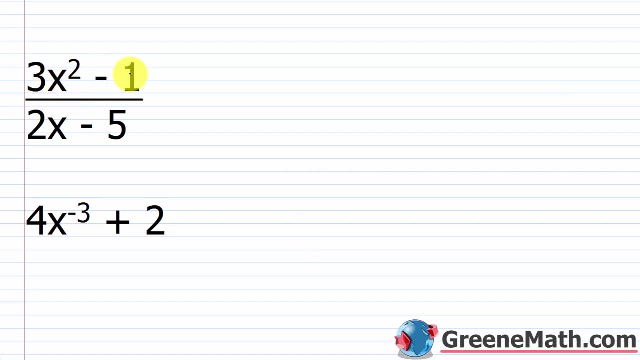 I'm good to go. Nothing is in the denominator, so we know that one is a polynomial. Now if I look at these two, they're not a polynomial. So 3x squared minus 1 over 2x minus 5 will have a. 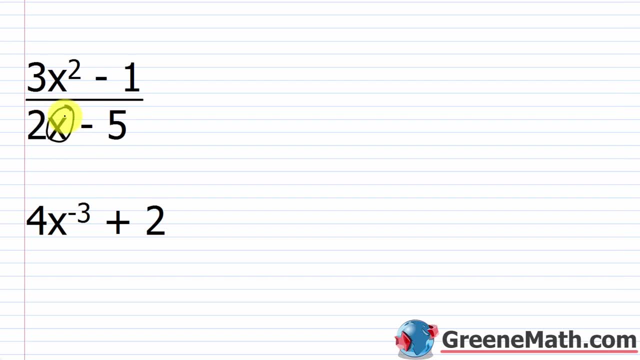 variable in my denominator and that violates the definition of a polynomial. This is in fact called a rational expression. We study those in Algebra 1 and we'll get to those pretty soon in Algebra 2.. But this is not a polynomial. This other example here: 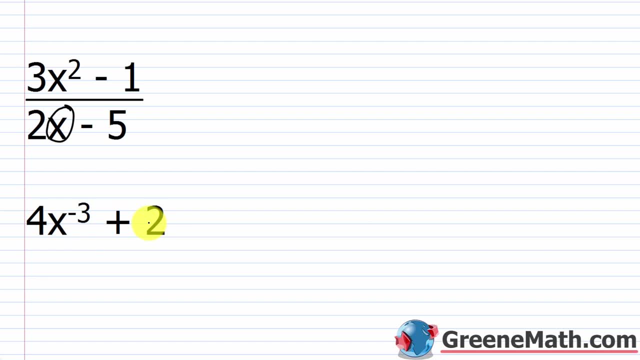 4x to the power of negative. 3 plus 2 is also not a polynomial, because we have this exponent of negative 3.. So negative 3 is not a whole number If you see something like negative something or you see a fractional exponent. 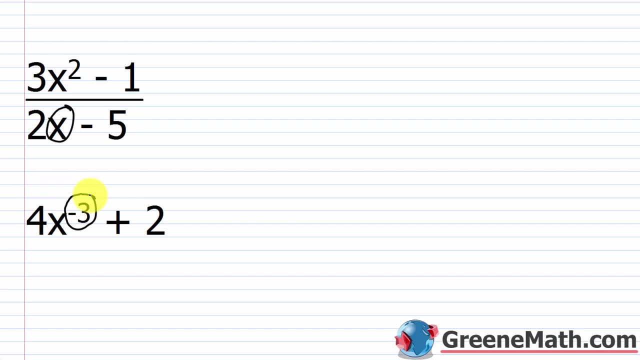 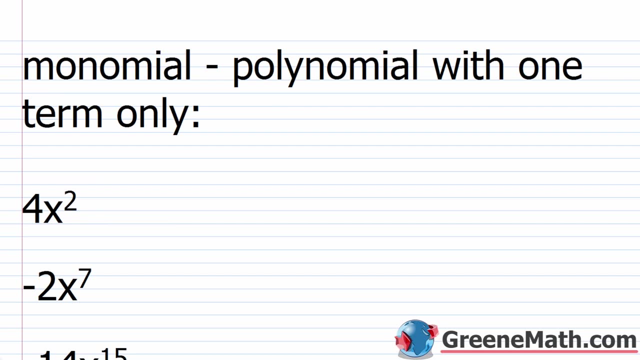 something like that. you don't have a polynomial Again. your exponents have to be whole numbers only. So we have three polynomials that occur so often that we give them special names. The first one is referred to as a monomial. 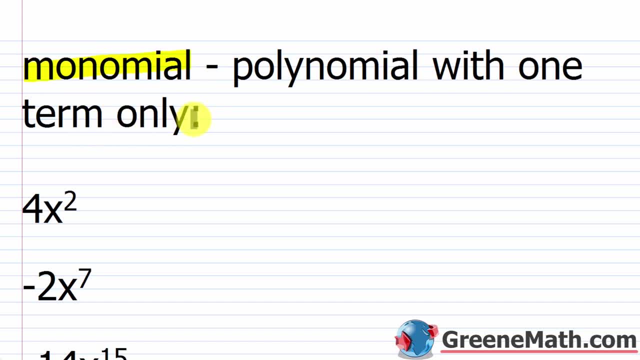 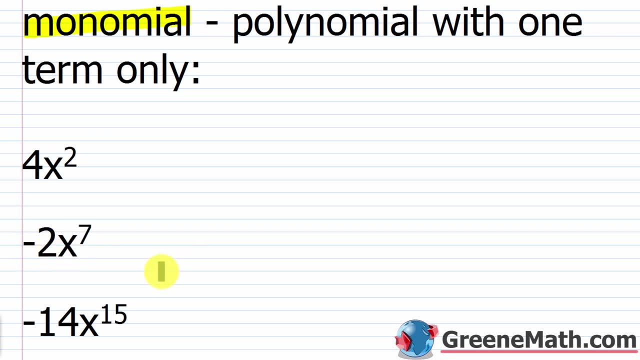 So this is simply a polynomial with one term only. So three examples: we have 4x squared, so that's a monomial negative 2x to the 7th power. that's a monomial and negative 14x to the 15th power. 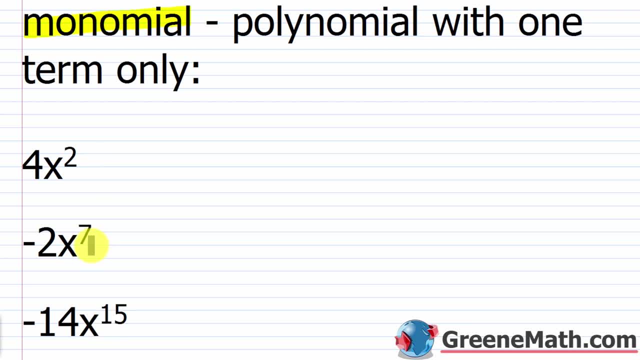 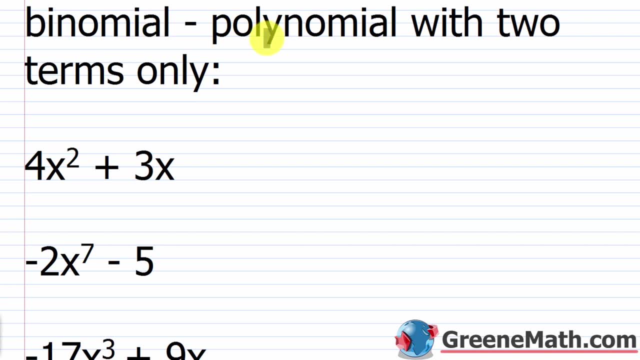 that's a monomial as well. So in each case we just have one single term, and that is the definition for a monomial. Alright, so the next one would be a binomial. So this is a polynomial with two terms only. Now again notice how the terms 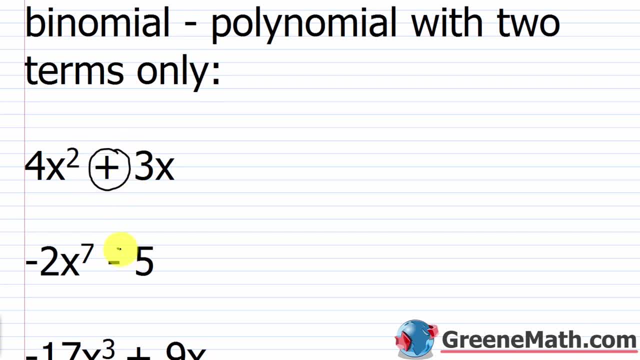 are separated by either a plus or a minus sign. So when you see one of those signs, you know you've separated two terms. So this is a term and this is a term. This is a binomial. I've got 4x squared plus 3x. 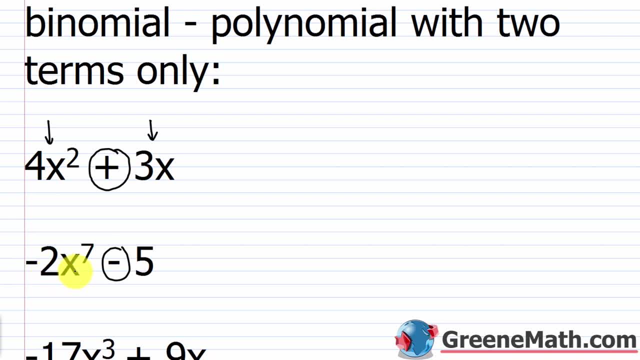 so that is a binomial. Then the same thing here. I've got negative 2x to the 7th power minus 5. So I've got a term here and a term here. The minus sign separates the two, So that's a binomial as well. 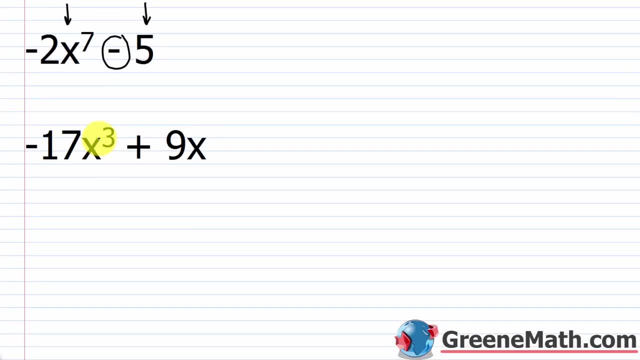 And then, as a final example, I have negative 17x cubed plus 9x Again. this is a term here. This is a term here. The plus sign separates the two. So we have two terms and that fits the definition of a binomial. 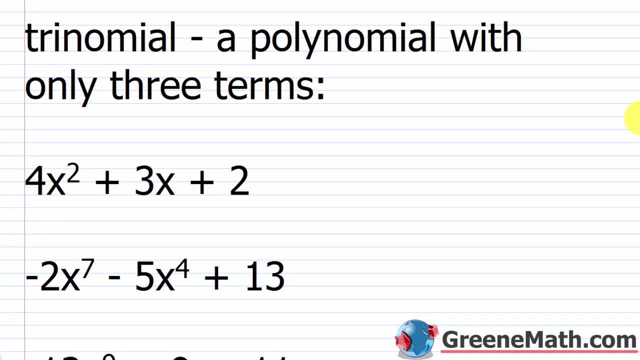 Alright. the next one we run across is called a trinomial. We think about a tricycle has three wheels. A trinomial has three terms. So a polynomial with only three terms is a trinomial. So we have an example here. 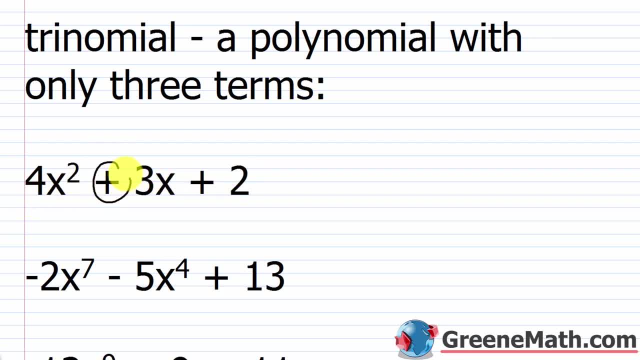 4x squared plus 3x plus 2.. Again, everywhere you see a plus or a minus sign, you're separating terms. So you have a term here 4x squared 3x And a term here of 2.. 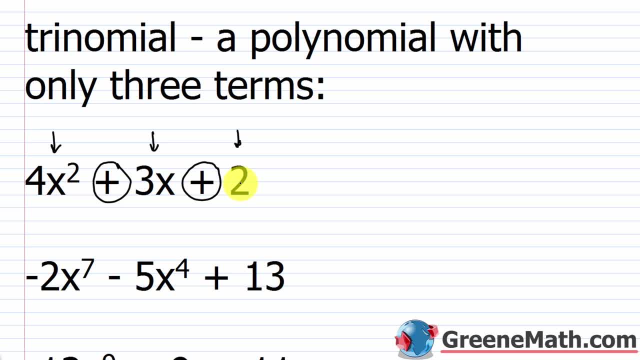 So 4x squared plus 3x plus 2 has three terms, and so it's a trinomial. Same thing here. I have negative 2x to the 7th power minus 5x to the 4th power plus 13.. 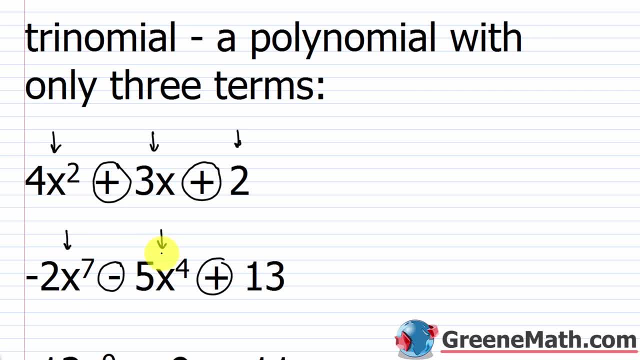 The minus sign and the plus sign separate the terms. So I've got a term here of negative 2x to the 7th power, a term here of 5x to the 4th power and a term here of 13.. That is a trinomial. 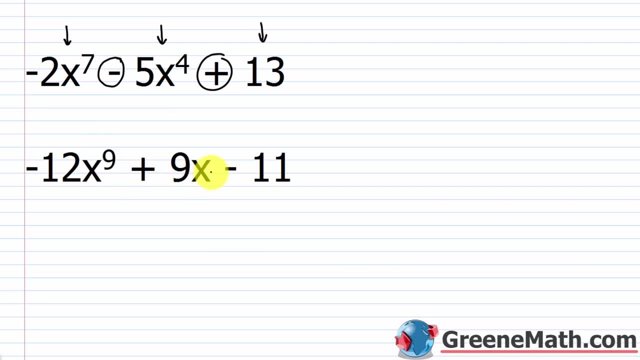 Alright. the last example is negative 12x to the 9th power plus 9x minus 11.. Again, this and this, the plus and the minus separate the terms. So I've got negative 12x to the 9th power. 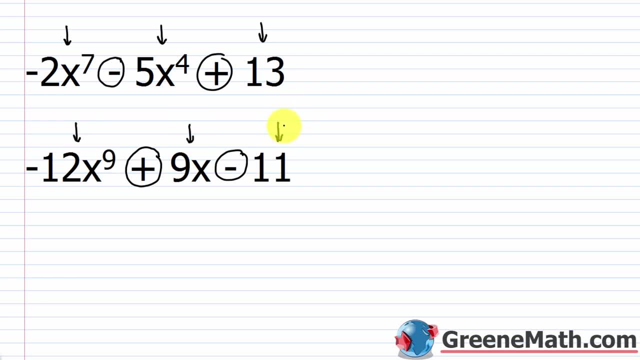 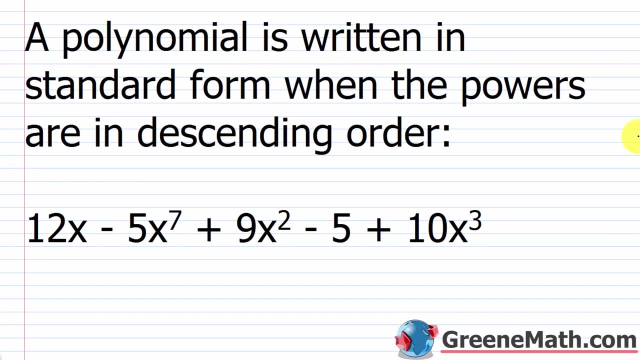 I've got 9x and I've got 11.. So three terms here in this polynomial. So this is a trinomial. Alright, so pretty easy stuff overall, Stuff that you would have learned in Algebra 1.. Here's another kind of common thing. 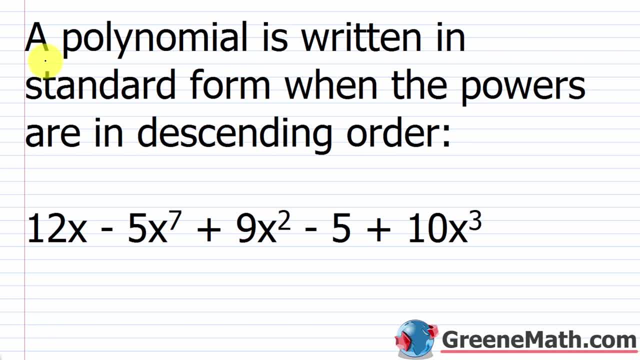 you need to know Standard form. So a polynomial is written in standard form. Let me just highlight that. So standard form when the powers are in descending order. So this is starting all the way to the left and working your way to the right. 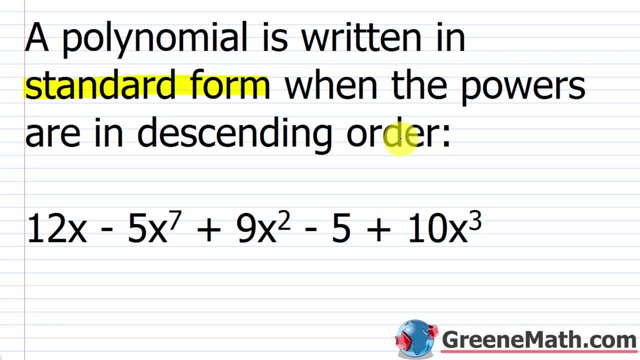 So I'm going to take the term that has the highest exponent on the variable and I'm going to put it all the way to the left, Then I'm going to go to the next highest, Then the next highest, So on and so forth. 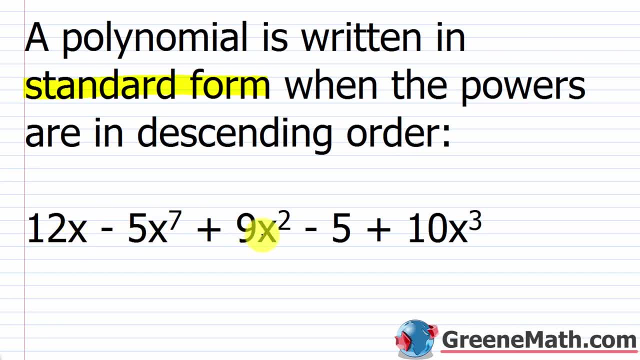 So if I look at this, 12x minus 5x to the 9th power plus 9x squared minus 5 plus 10x cubed, our variable is x. What is the highest exponent on this variable? Well, it's this: 7 here. 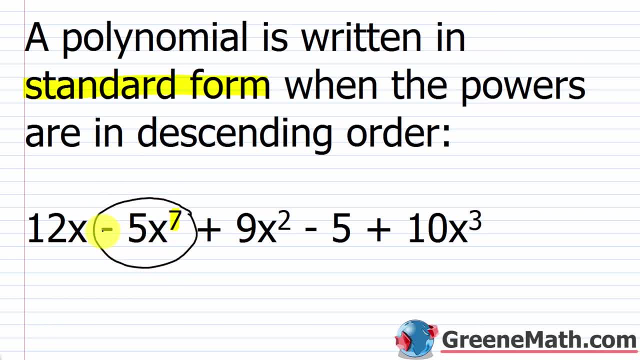 So I want to write this term right here and I've got to include that negative, the negative 5x to the 7th power. I want to put that all the way to the left, So if I put equals negative 5x to the 7th power. 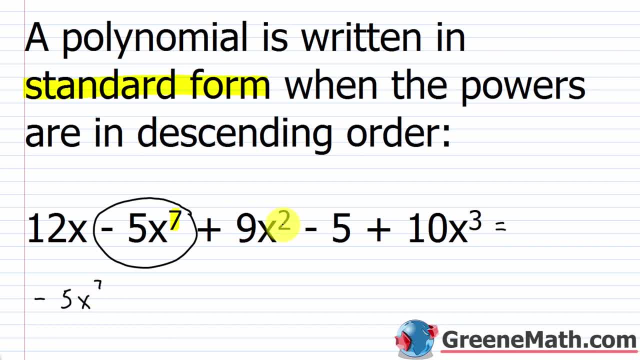 then I would say: what is the next highest exponent? Well, this one's a 2, this one's a 3 and this one's understood to be 1, so I would go with this 3 here. so this term, 10x cubed would come next. 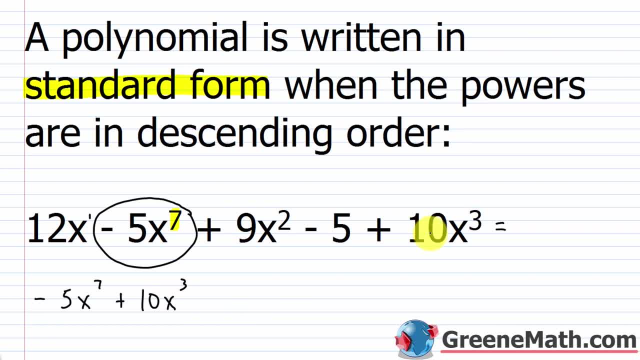 So plus 10x cubed, then I'd put plus 9x squared, that would be next. then I'd put plus 12x, that would be next, and then this constant here, negative 5, would be all the way at the end. So this: 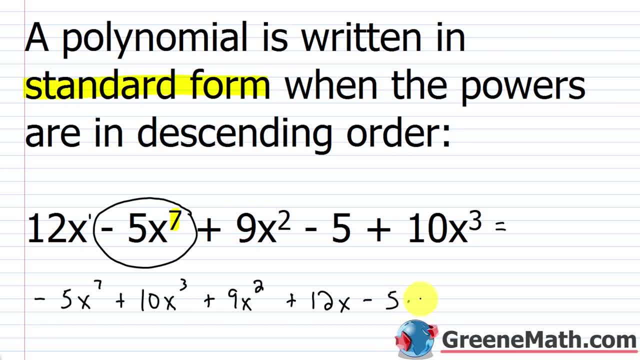 we could think of as being multiplied by x to the power of 0. You might see that in a textbook and be very confused. you might say: why would they do that? So x to the power of 0 is understood to be 1 again, as long as x is not 0. 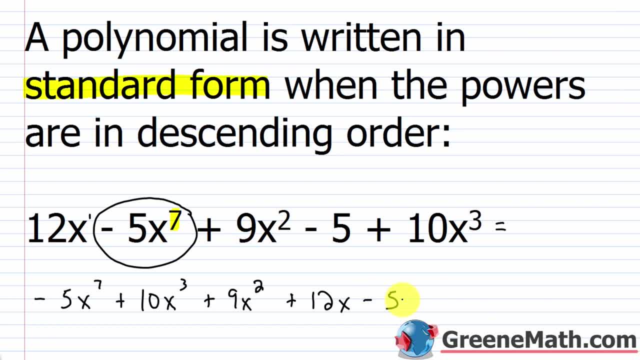 So negative 5 times 1 is just negative 5. so really I haven't changed anything there. it's just a neat little trick to put a variable next to it. So in standard form this polynomial is read as negative 5x to the 7th power. 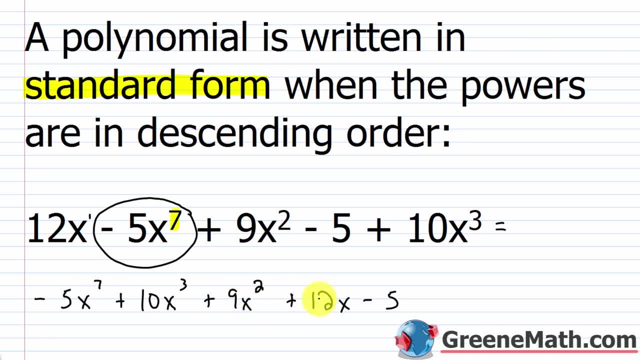 plus 10x cubed plus 9x squared, plus 12x minus 5, and again you can notice how your exponents go in descending order. you've got 7,, 3, 2. this would be a 1, and again. if you wanted to, you could write this: 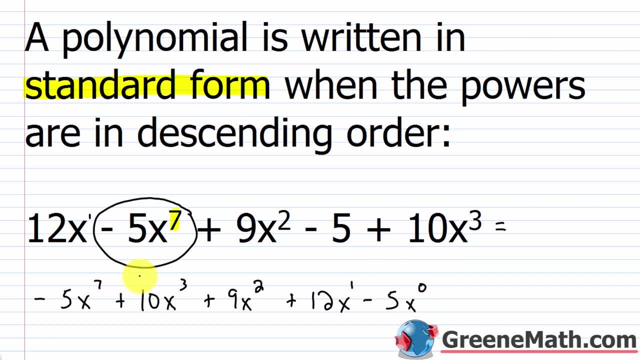 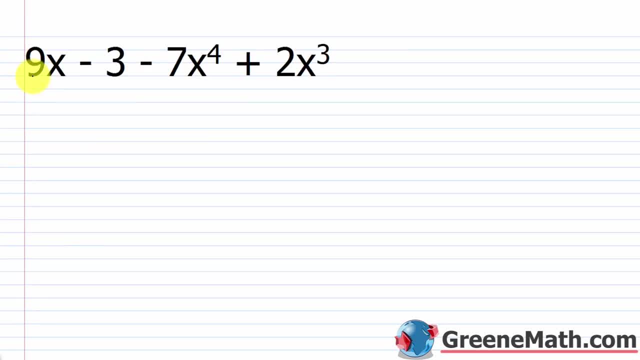 as having an exponent on x of 0, so 7,, 3,, 2,, 1 and then 0, so in descending order. alright, so let's take this one and write it in standard form. we have 9x minus 3 minus 7x to the 4th power. 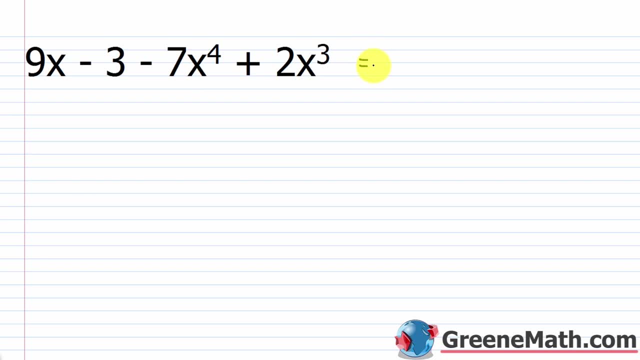 plus 2x cubed. so the highest exponent on the variable x occurs right here. so I've got to take that negative and bring it with me, ok, so I'm going to put negative 7x to the 4th power. and you might ask yourself: 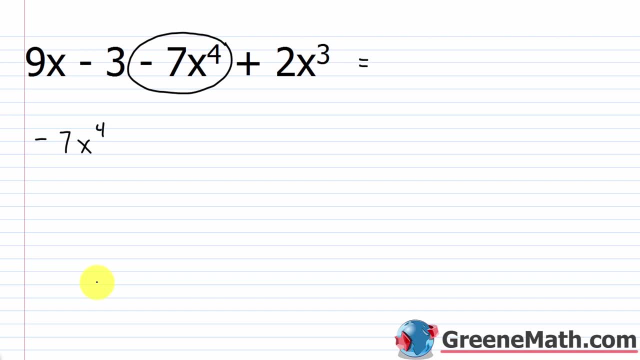 if you're not familiar with a lot of things, why am I taking that negative with me? remember, you can rearrange things with addition, but not with subtraction. ok, so if I put this as plus negative 7x to the 4th power, I just bring the negative with me. 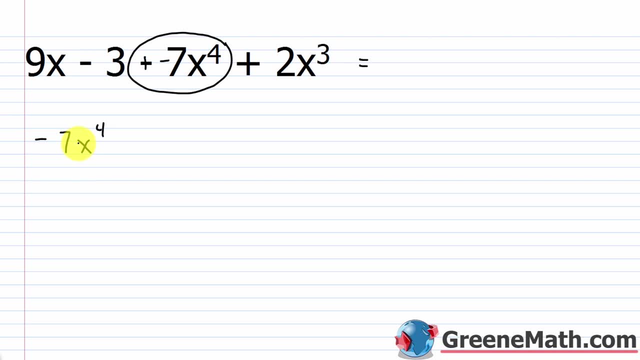 and I can rearrange things as much as I want. if I just took things as they were and I just moved this over here and I didn't put my subtraction over there and I just left the signs where they were, you'd have a problem there, and I can't just move this over here. 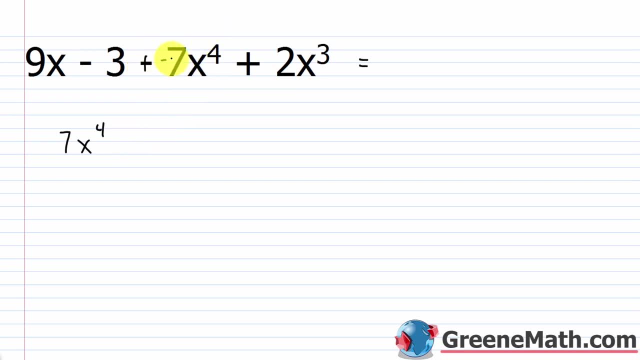 and leave the sign where it is. so I change this to plus negative and you can do it without doing it and just put a minus 7x to the 4th power, so there's no problems there. now the next thing we want to think about is: 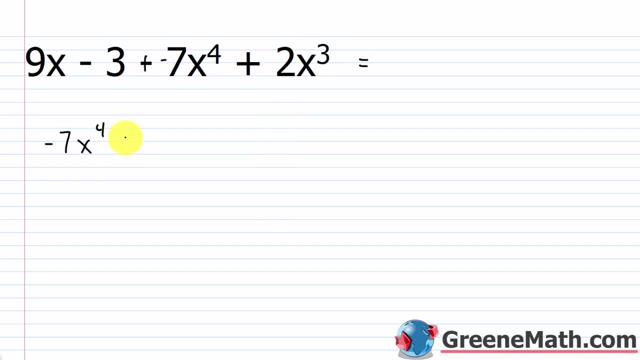 2x cubed, because the exponent there is a 3. so then plus 2x cubed, and then next I want plus 9x, because the exponent there would be a 1, and lastly I just want that constant negative 3, or you can think about it as just minus 3. 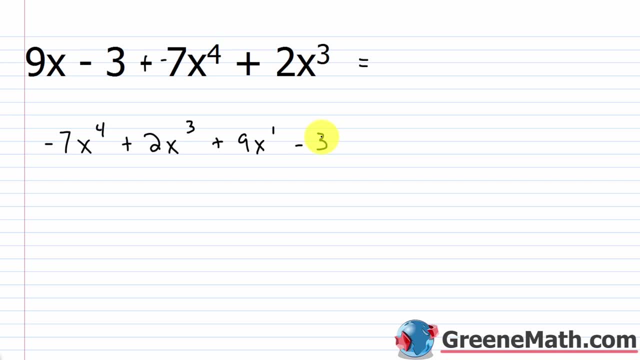 alright, so I've rearranged everything to where the exponents are in descending order: a 4, a 3, a 1, and again you could write this as negative 3 times x to the power of 0, so then you could say you have a 0 here. 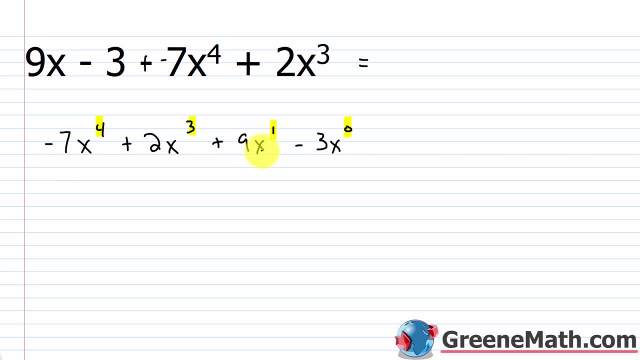 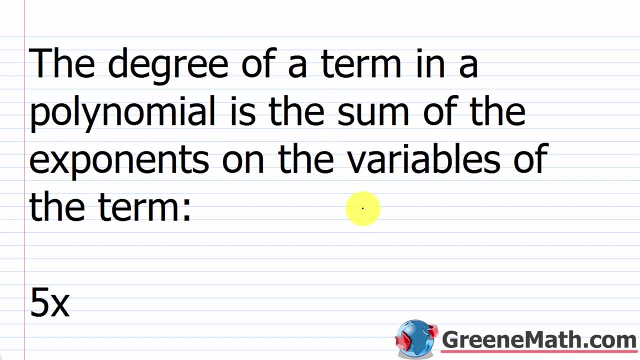 so negative 7x to the 4th power, plus 2x cubed, plus 9x, minus 3 x to the power of 0, or you could just put minus 3, alright, same thing. so the last thing we're going to review is called the degree. 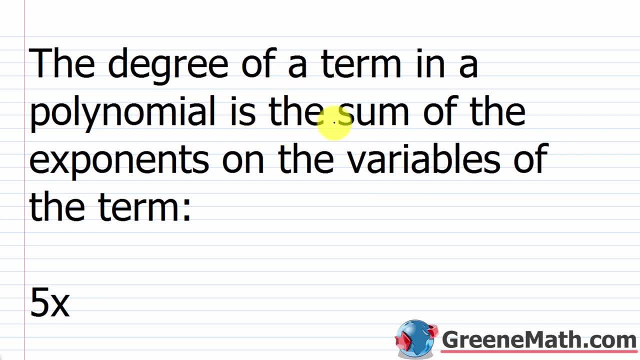 so the degree of a term in a polynomial is the sum of the exponents of the variables of the term. so all I'm going to do to find the degree is look at the exponent, or it could be exponents if you have more than one variable. 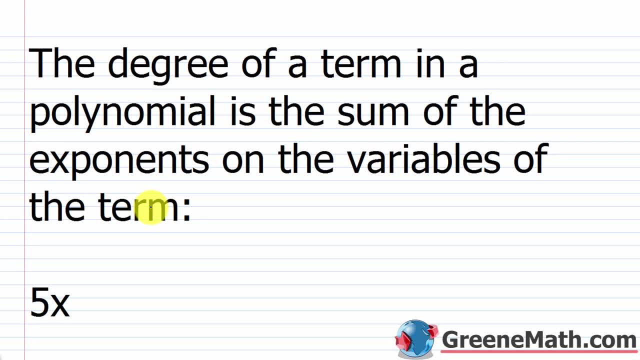 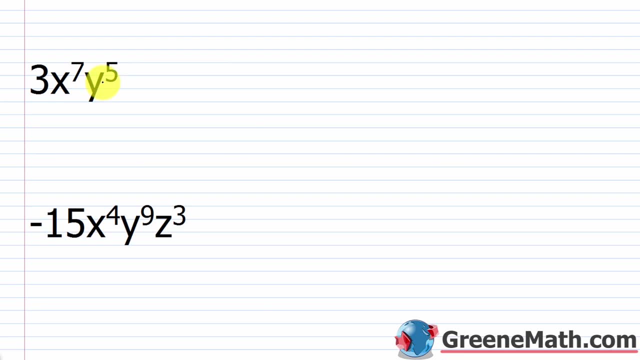 and whatever the sum is, that's the degree of the term. so in other words, with 5x- we know the exponent here is understood to be 1, so the degree is 1 for this example: 3x to the 7th power, y to the 5th power. 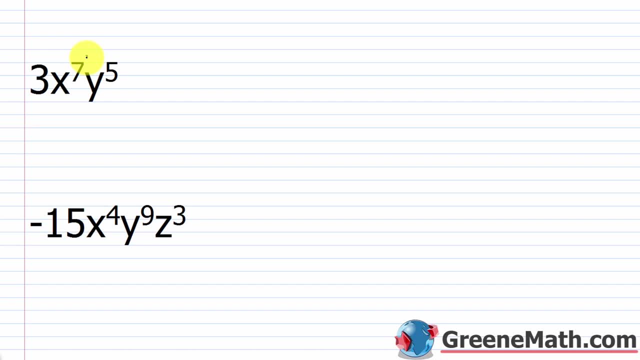 we have two variables involved, so what I want to do is some addition. I have an exponent of 7 and an exponent of 5. 7 plus 5 is 12, so the degree is 12. so this isn't very difficult at all. it's just something you kind of need to know. 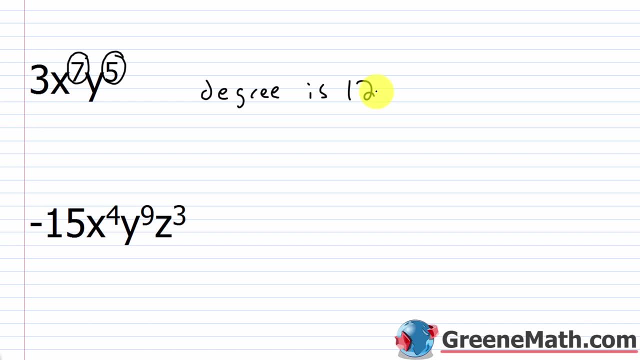 once you know it and you understand the definition. it's very, very simple for this one negative 15x to the 4th power, y to the 9th power, z, cubed again, I'm just going to add the exponents: 13 plus 3 is 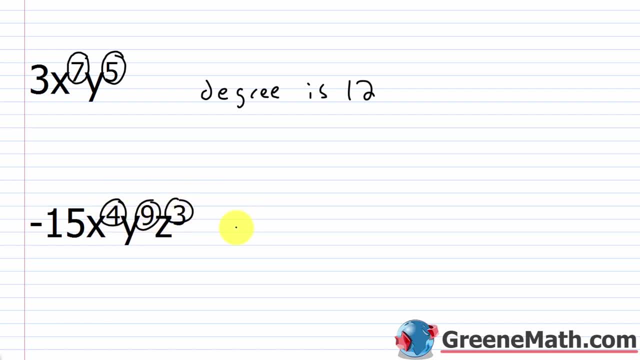 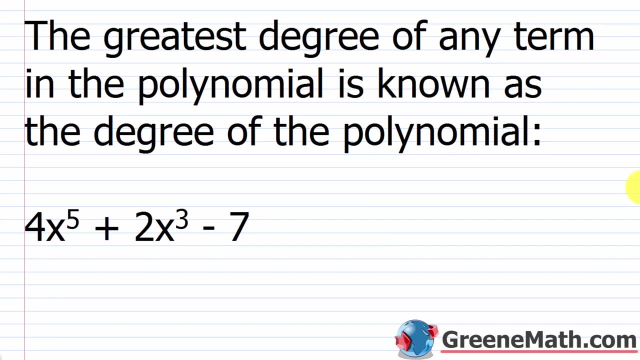 16. so this plus this, plus this, your degree is 16. alright, so let's extend this a little bit further. now we're going to talk about the degree of the polynomial itself. so the greatest degree of any term in the polynomial is known as the degree of the polynomial. 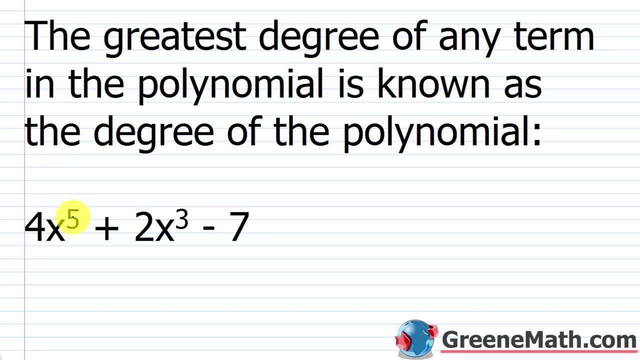 so as an example here I have 4x to the 5th power plus 2x cubed minus 7, so I would look at each term individually. so for this term here the exponent is 5, so the degree of that term is 5. 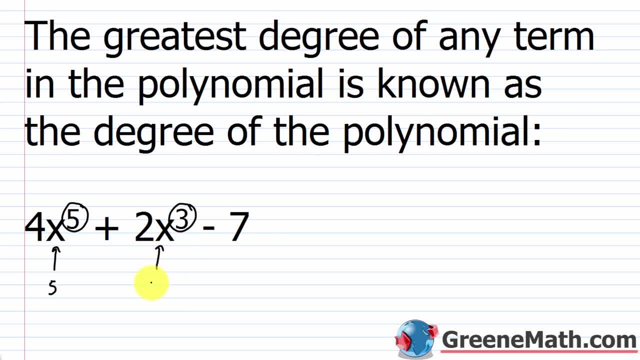 then this term: here 2x cubed. the exponent is a 3, so the degree of the term is a 3. and then for this negative 7, again a little trick: here. I can write x to the power of 0 next to it. I showed you that earlier. 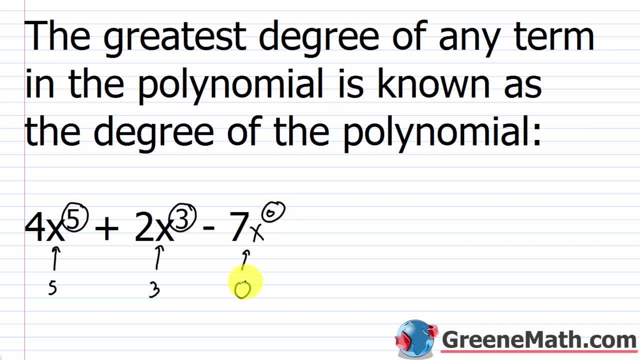 so the degree for this would be 0. now, which term has the highest degree? well, this one does so, since the degree for that term is a 5, that means the degree of the polynomial is a 5. this polynomial has a degree of 5. alright, let's take a look at another one. 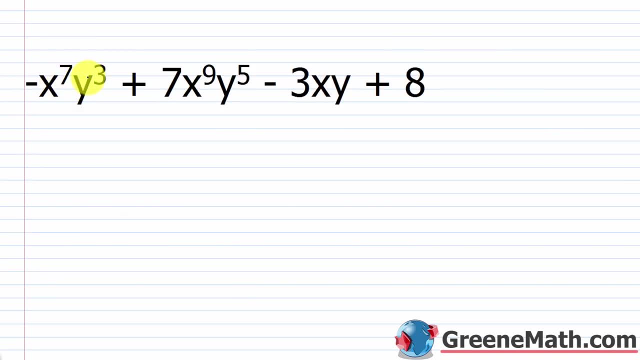 so we have negative x to the 7th power y cubed plus 7x to the 9th power y to the 5th minus 3xy plus 8. so again, I want to look at each term individually. to start, if I look at this term here, I have: 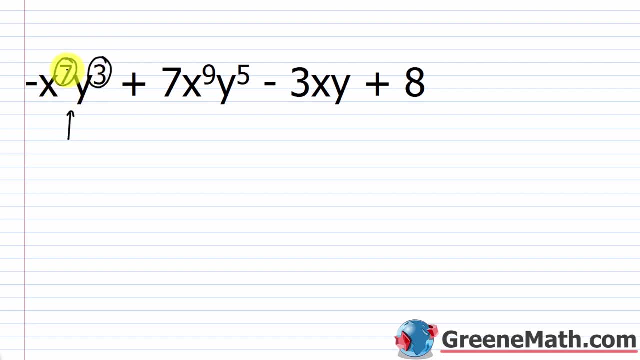 7 as an exponent and a 3. I've got to sum those two. so 7 plus 3 is 10. for this one, I have a 9 and a 5. 9 plus 5 is 14. for this one, I have a 1. 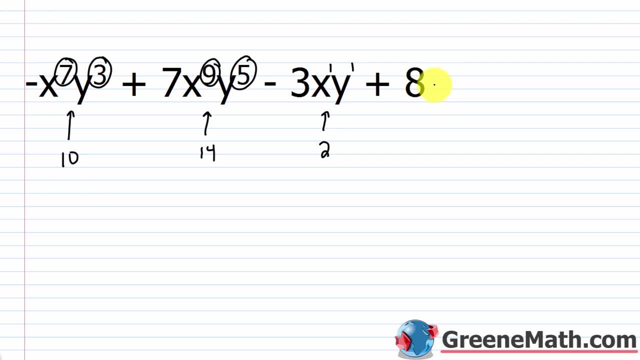 and a 1. 1 plus 1 is 2, and then for this 8- here I can write this as times x to the power of 0. so this is 0 in general. when you look at a constant, the degree is 0. now the only exclusion to that. 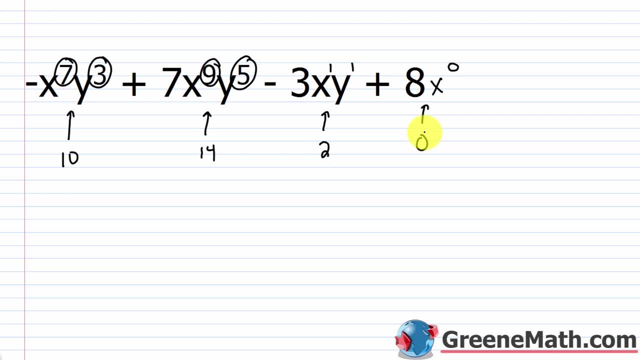 is the number 0 itself, but anything other than 0. if it's a constant, it's going to have a degree of 0. so if I think about this polynomial here, we see that this is the big winner this term right here. so the degree for this is 14. 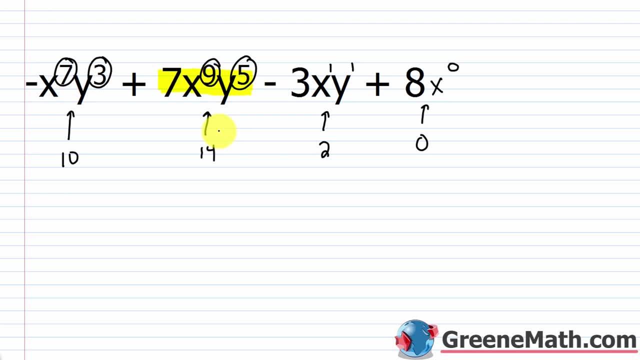 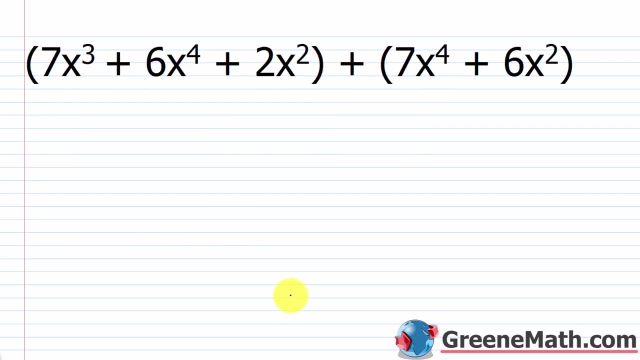 so the degree for the polynomial is 14. so the degree is 14, alright, so now that we've kind of reviewed some of the things that we need to know, let's jump in and start adding and subtracting polynomials. so for the majority of you, you've already done this. 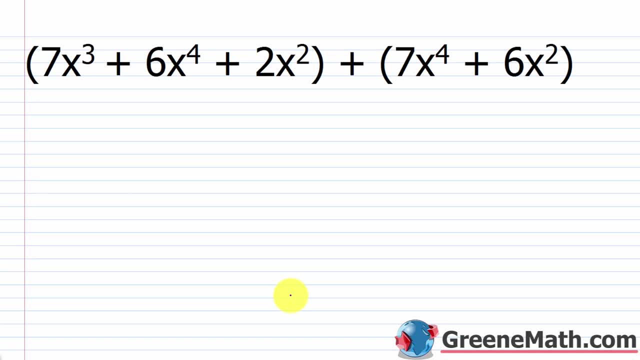 this is a review and you remember how easy this is. the only thing you have to really get down here is the concept of like terms. so like terms have the same variable, or it could be variables if we have a harder problem and they're raised to the same. 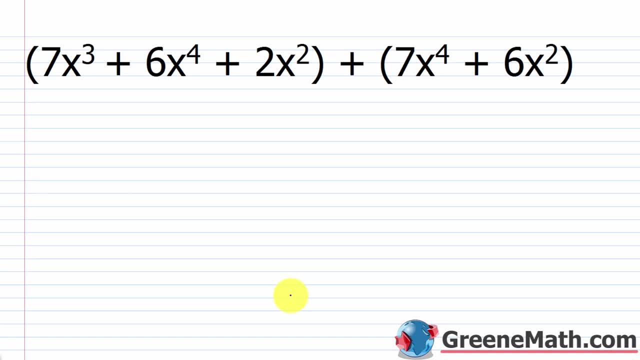 power or it could be powers. so, as an example, if I have something like 2x to the third power and I have 3x to the third power, what are like terms, the coefficients or the number parts here don't matter. don't pay attention to that when you're trying to find like terms. 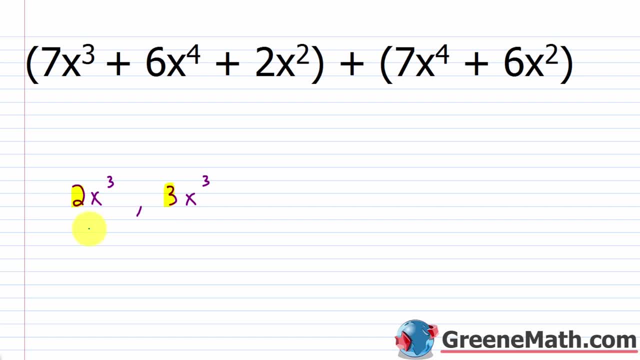 you just want to make sure that the variable is the same, so I have an x here and an x here, so that's good to go. then I want to make sure my exponent is the same. I have a cubed and I have a cubed, so that's the same. 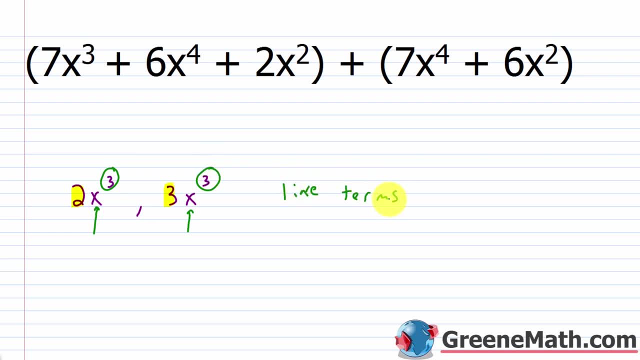 so these are like terms. and how do we go about adding like terms? well, if I had something like 2x cubed plus 3x cubed, all I need to do is add the numerical coefficients. so 2 plus 3, which is 5. 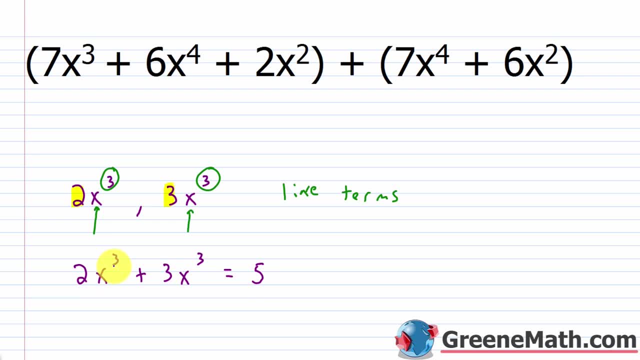 and then the x cubed part stays the same times x cubed. you can think about it as having 2 apples plus 3 apples gives you 5 apples. but if I wasn't adding like terms, let's say I was adding oranges and apples. well, 2 apples plus 3 oranges. 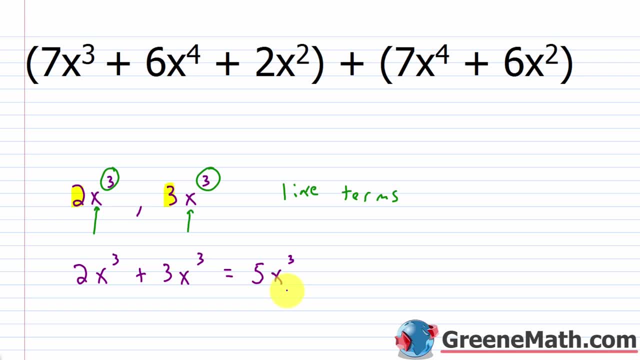 is just 2 oranges and 3 apples. I can't really make that simpler. so as an example of something that's not like terms, let's say that we had 2x cubed, and let's say 3y to the 4th power. 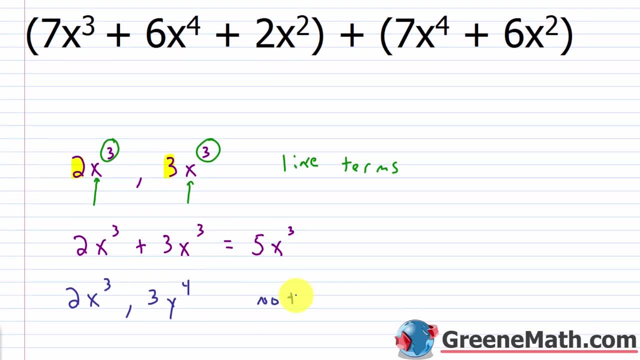 well, these are not like terms. these are not like terms. why is that the case? well, I have an x here and I have a y here, so the variables are different. the exponents are also different. I have a 3 here and a 4 here. if the exponents were the same? 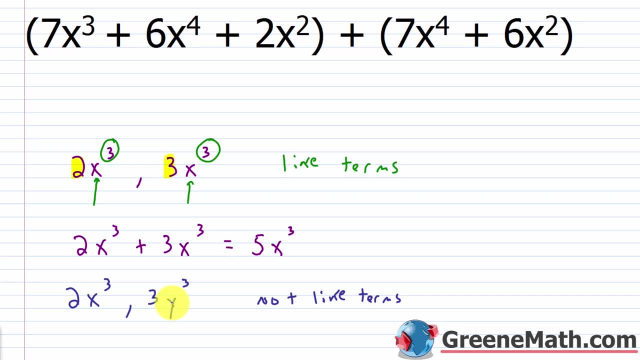 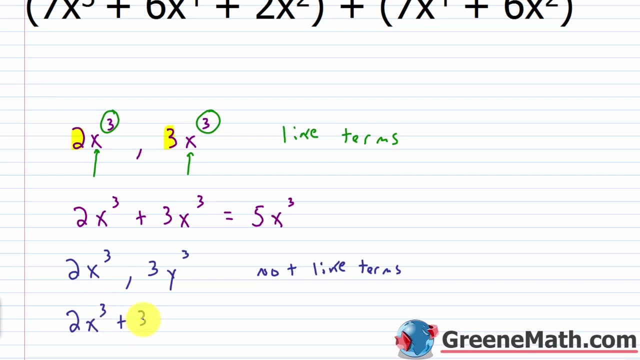 it doesn't matter, it needs to be the same variable raised to the same power. so that's how you have like terms. so if I added 2x cubed and 3y cubed, you can't combine that or make that any simpler. there's nothing you can do. 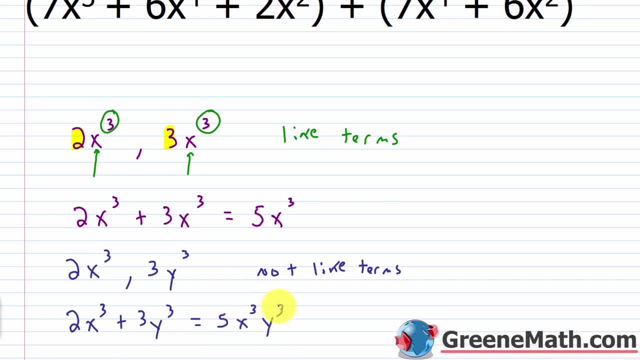 and a lot of students make the mistake and say this is 5x cubed, y cubed. you can't do that. that's wrong. this is wrong. it's important that you understand that. you can only combine like terms, alright, so let's erase all this. 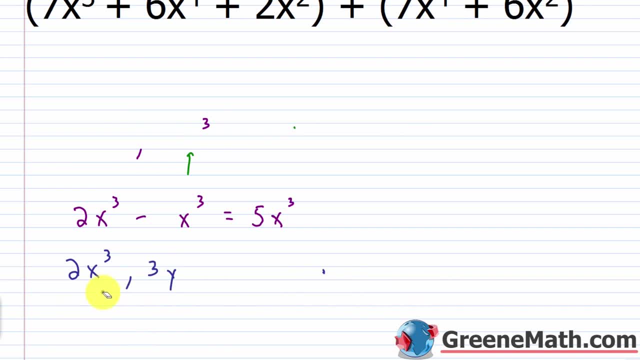 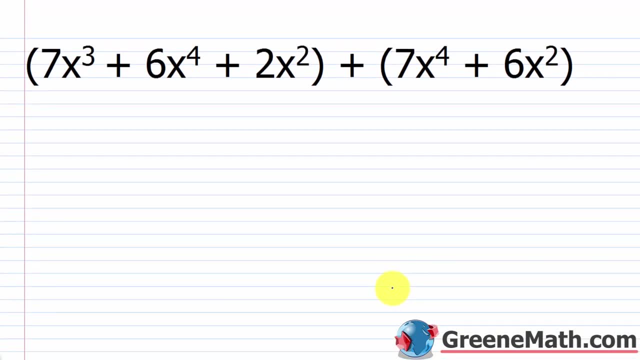 I think all of you pretty much understand this at this point. if you don't, as we're working through the examples, I think you'll easily pick this up. so I start out with adding this polynomial here: 7x cubed plus 6x to the 4th power. 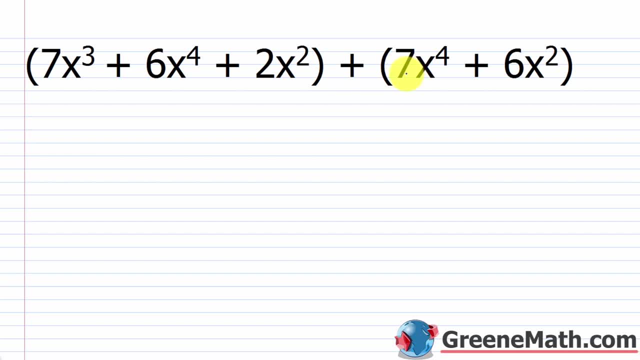 plus 2x squared, and we're adding to this the other polynomial, 7x to the 4th power, plus 6x squared. the first thing is I can just drop parentheses. I don't really need them, so I can write this problem as 7x cubed. 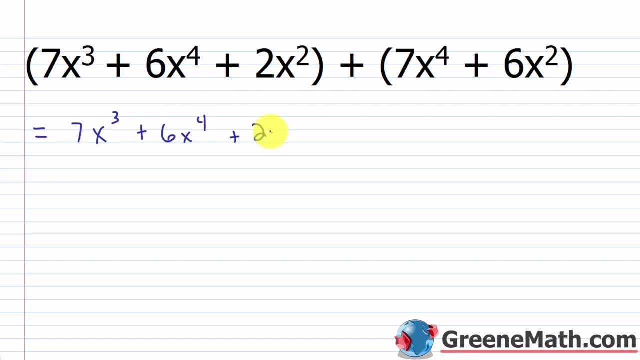 plus 6x to the 4th power plus 2x squared. plus 7x to the 4th power plus 6x squared. now the next thing that I like to do, and I don't do this anymore, but when I started, my teacher told me this: 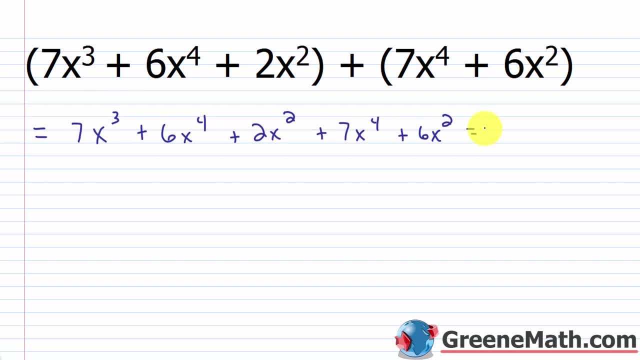 and I loved doing it when I was struggling. I want to look for like terms right away and I want to write them next to each other and it's obvious what I need to do. so, in other words, if I start out with 7x cubed, 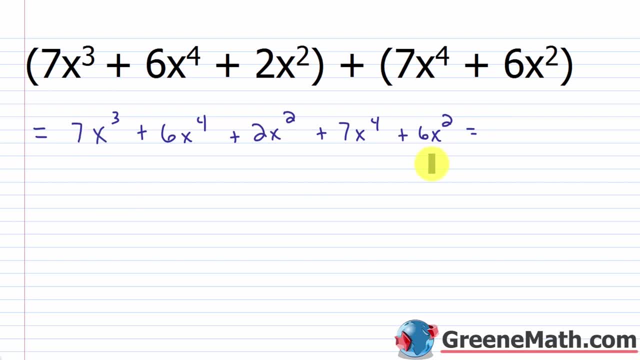 do I have another term with an x cubed in it? no, I do not, so I don't need to do anything there. I have 6x to the 4th power. next, do I have another term where I have x to the 4th power? 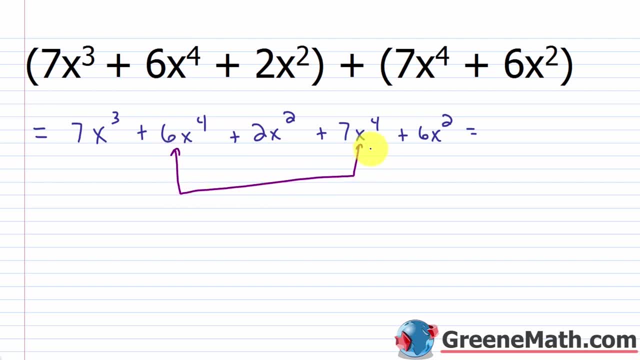 yeah, I have this one and this one. then I have 2x squared. do I have another term with x squared? yeah, this one and this one. so let's reorder this. I'm going to put 6x to the 4th power in the very front position. 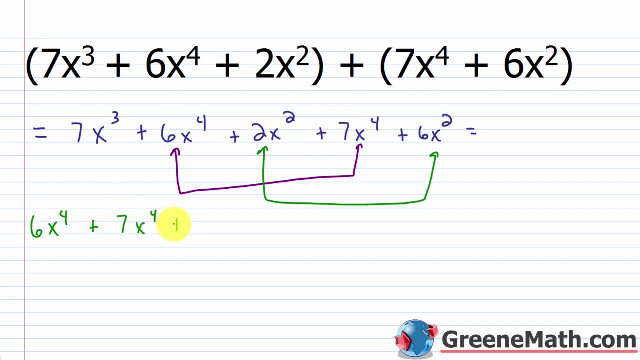 then plus 7x to the 4th power, then plus 7x cubed, then plus 2x squared, then plus 6x squared. now I did two things there. the first thing is I took the exponents that were highest and moved them to the left. 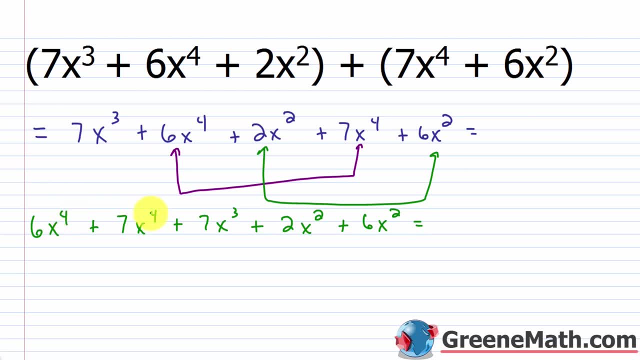 and I went in descending order. so this is the exponent with a 4, a 4, a 3, then a 2, then a 2, so it's in descending order. so when I get my answer it's going to be in standard form. 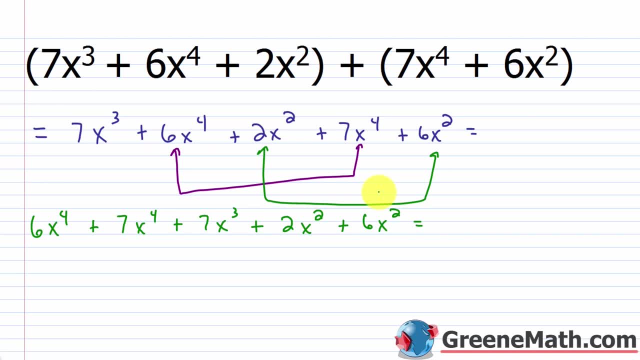 so that's the first thing I did. the second thing I did was I arranged it to where like terms were next to each other. so these are like terms and these are like terms. so now all I got to do is add the coefficients, keep the variable part the same. 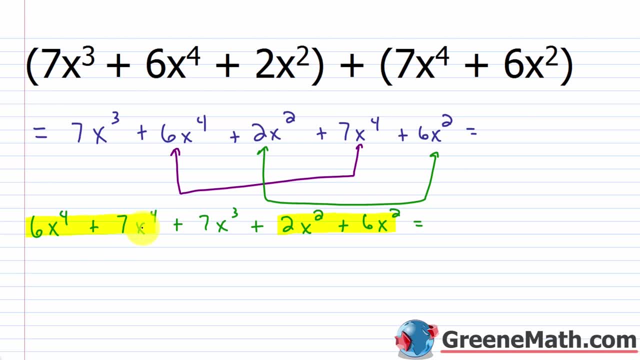 so 6x to the 4th power plus 7x to the 4th power. add 6 plus 7, that's 13, and x to the 4th power just stays the same. if I had 6 apples and 7 apples, 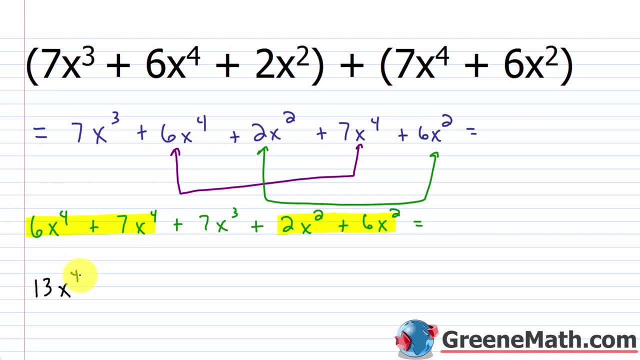 if I added them I would have 13 apples. so then plus, we have 7x cubed, and then plus. now we have like terms again. we have 2x squared plus 6x squared. 2 plus 6 is 8, and then x squared comes along for the ride. 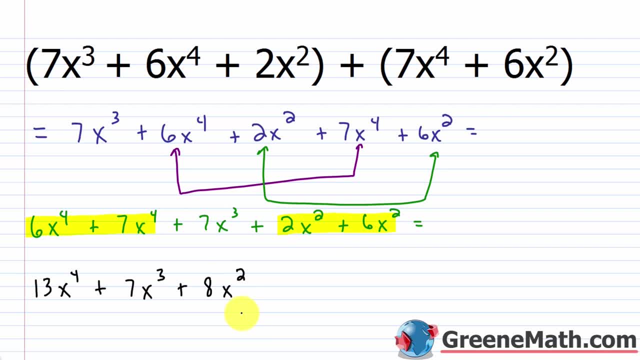 now. there's no way to make this any simpler. we simply don't have any more like terms. our variable is the same in each case, but the exponents are different. this is like adding apples, oranges and nectarines. ok, if I had 13 apples plus 7 oranges. 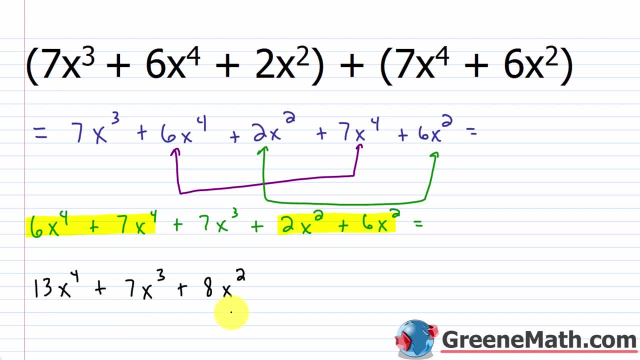 plus 8 nectarines. I can't really make that simpler. if I had 13 apples and 7 apples, I could just say I have 20 apples. so that's kind of a real world example of what we're going through here. so our answer is just 13x to the 4th power. 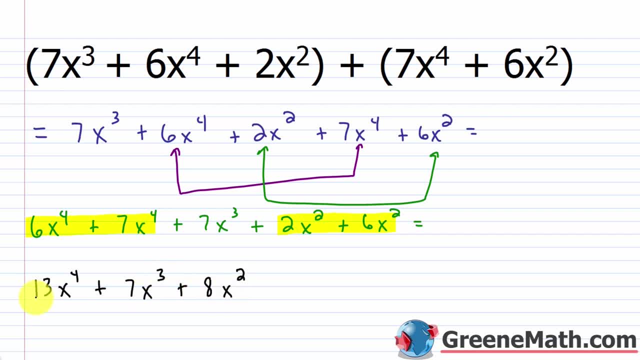 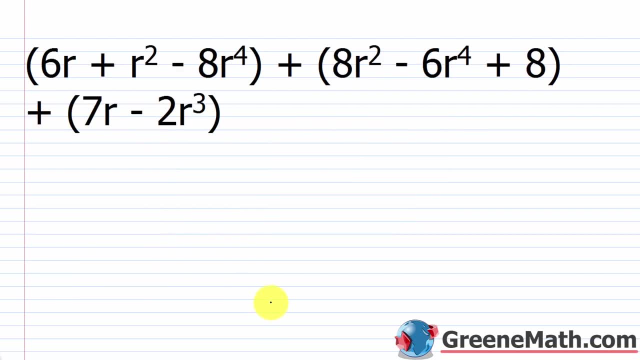 plus 7x cubed, plus 8x squared. and again, notice how it's written in standard form you have x to the 4th x cubed and then x squared. alright. as a next example, we have plus r squared, minus 8r to the 4th power. 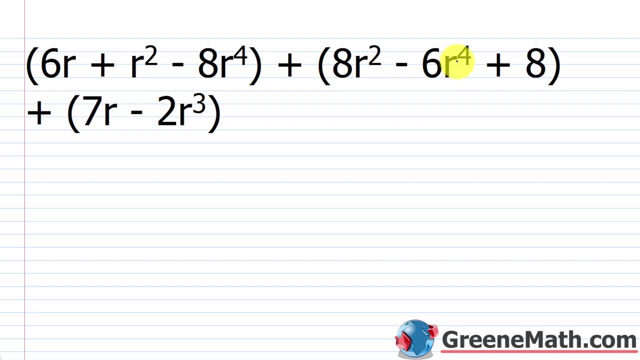 then plus 8r, squared minus 6r to the 4th power, plus 8, then plus, we have 7r minus 2r cubed. alright. so the first thing I want to do again is reorder these things. I'm going to start out with negative 8r to the 4th power. 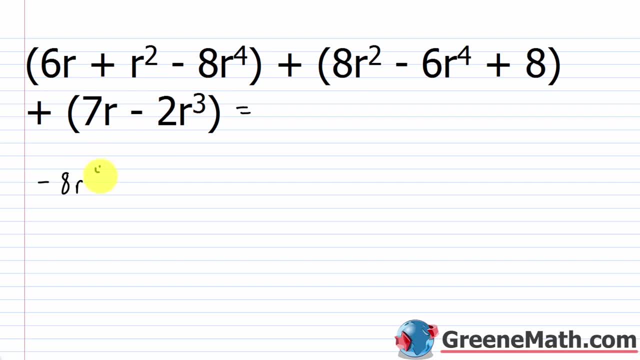 so negative 8r to the 4th power. remember, I'm taking this sign with me. I can think about this as plus negative 8r to the 4th power, and then over here I see I have negative 6r to the 4th power. 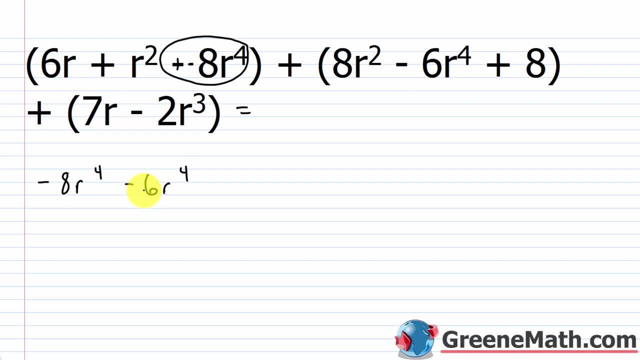 so I write those two next to each other again. why did I start out with that? because, as I scan through here, the highest exponent on r is a 4, so that's why I chose to put this all the way to the left. now I'm going to scan through and see: do I have r cubed? 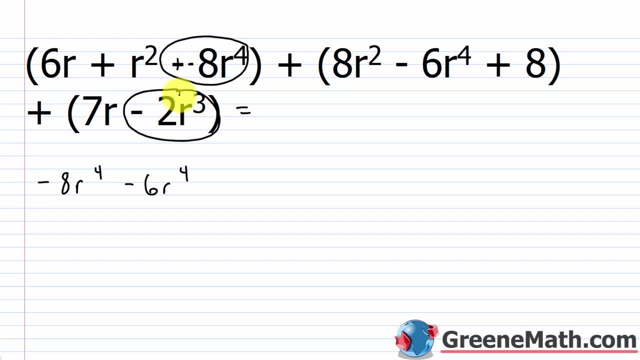 yeah, I've got one right here, so again the sign comes with it. I'm going to write negative 2r cubed, and the next thing I'm going to look for is r squared. so I've got that here and here, so I'm going to put plus r squared. 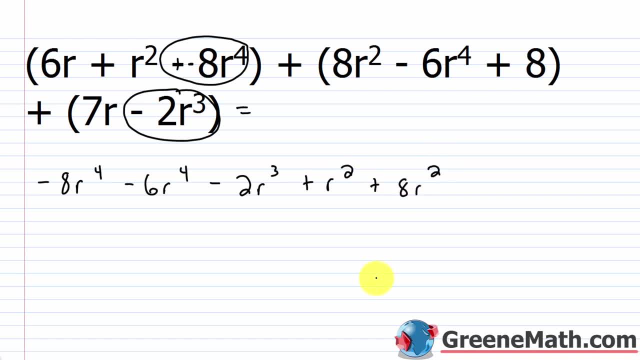 then plus 8r, squared. now I'm looking for r to the 1st power, and so that's 6r and 7r, so plus 6r, plus 7r. and then, lastly, I have this: plus 8, so plus 8. 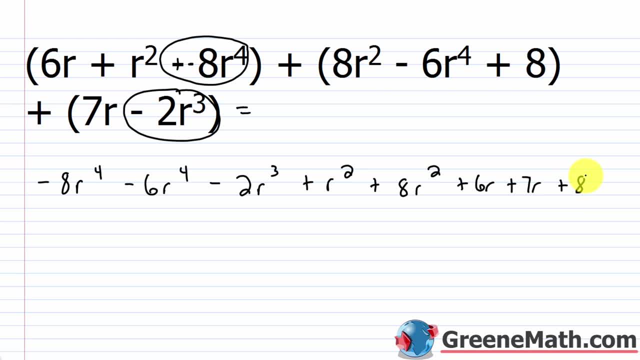 now one of the things you might want to do, especially when you first start out. you might write everything and you might miss a term. oh, I forgot that one. it's very, very common you might kind of go through, especially if you're on an important test, and check. 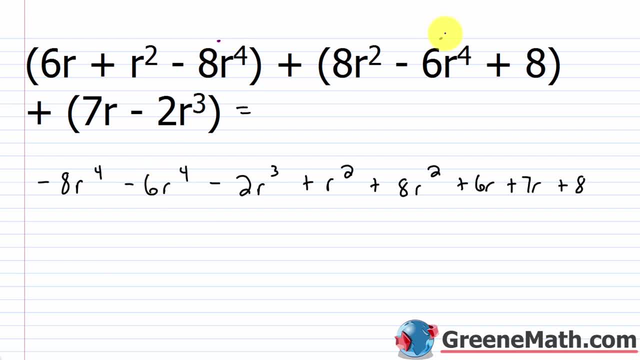 ok, I've got negative 8r to the 4th power. so I've got that negative 6r to the 4th power. so I've got that negative 2r cubed. I've got that r squared. I've got that 8r squared. I've got that. 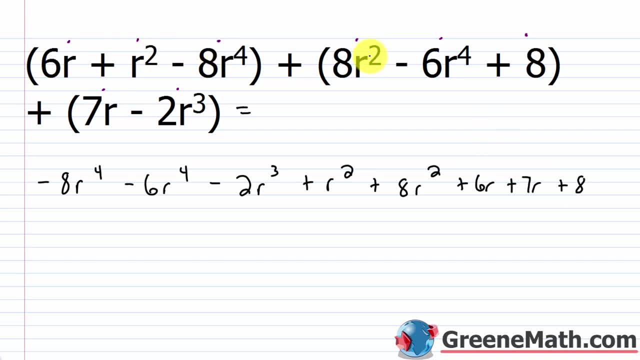 6r, I've got that, 7r, I've got that, and then 8, I've got that. you can go through and say: ok, I've got a dot there, there. there important that you put everything in there, otherwise you're not going to get the right. 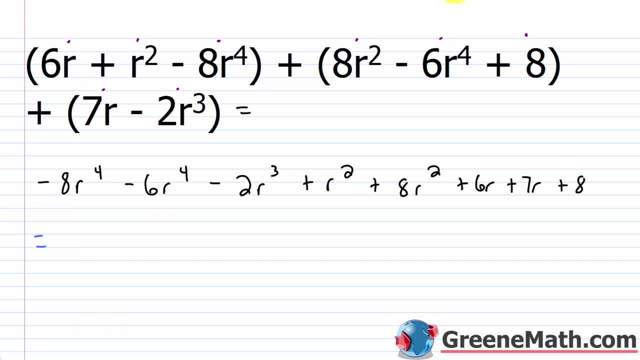 answer. So once we've set this up, we're just going to combine like terms. We've got like terms here and here and here. So negative 8r to the fourth power minus 6r to the fourth power is going to be negative 14r to the fourth power. Then we've got minus 2r cubed, then plus. 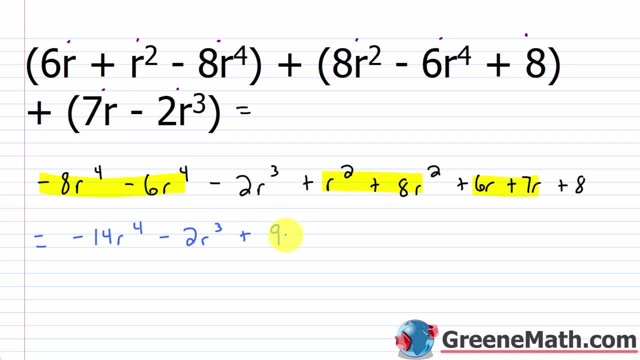 you've got r squared plus 8r squared, which is 9r squared, Then plus 6r plus 7r is 13r, then plus 8.. So it's just as easy as that and a lot of times moving forward, you're not even 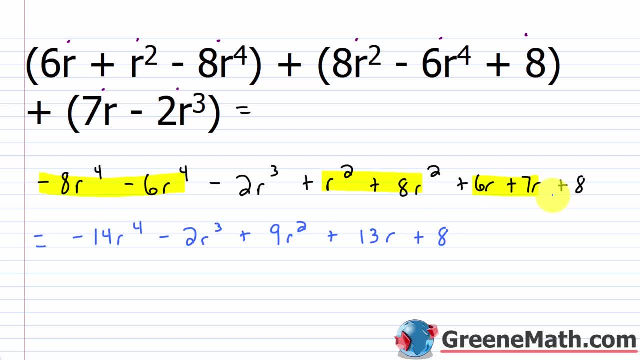 going to write this stuff out. Once you get good at this, you're just going to say: okay, well, negative 8r to the fourth power, minus 6r to the fourth power, write my answer- negative 14r to the fourth power- and just kind of go from there. I add these now just kind of mentally and just 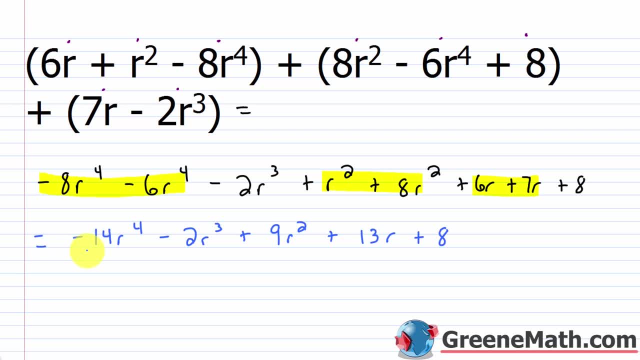 write them down. So I'm going to write them down. So I'm going to write them down. So I'm going to write down the answer. I don't advise that until you get really good at this, because it's very easy to make a mistake. Okay, so just start out with it, slow progress until you fully understand it and 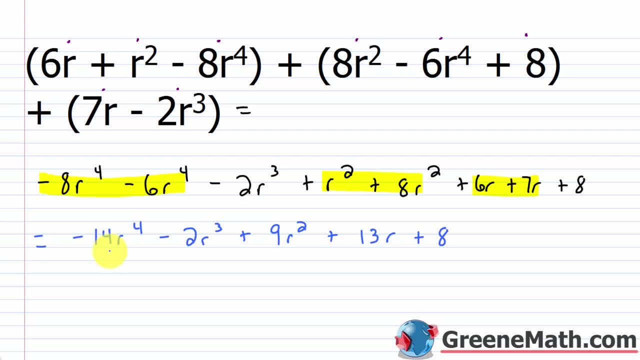 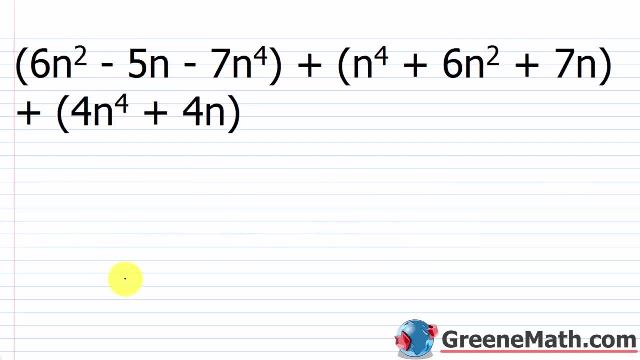 then you can try to do it just a little bit faster. So our answer here is negative: 14r to the fourth power minus 2r cubed plus 9r squared, plus 13r plus 8.. All right, so the next one is going to. 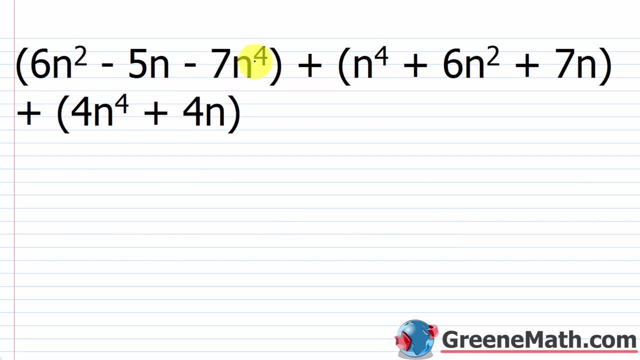 be 6n squared minus 5n, minus 7n to the fourth power, then plus n to the fourth power, plus 6n squared plus 7n, then plus 4n to the fourth power plus 4n. So I scan through this and: 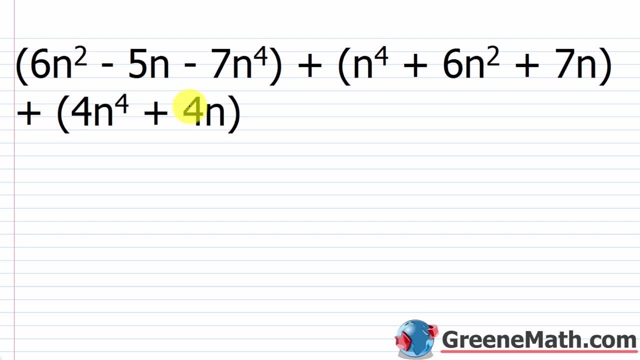 I see that 4 is the highest exponent. So what has a 4 as an exponent? So this term, this term and this term. So let's put equals. I'll start out with negative 7n to the fourth power. Again, take the negative sign with you, Plus n to the fourth power. I'll do that next, Then plus. 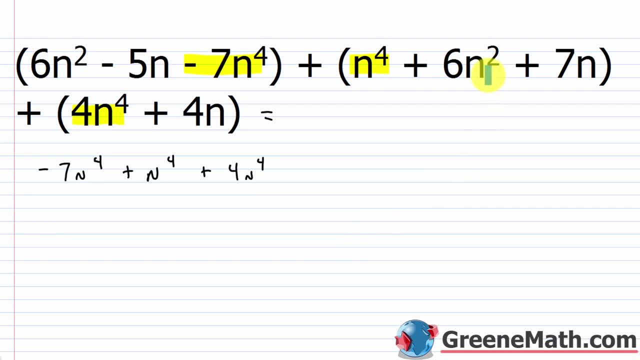 4n to the fourth power. Now the next highest exponent would be a 2.. I've got 6n squared, I've got 6n squared again, and that's all I've got. Let's write those. So, plus 6n squared, plus 6n. 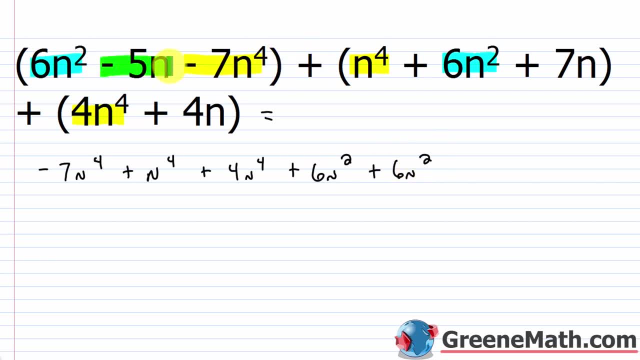 squared again. Then I've got my n to the first power. So I've got minus 5n and I've got plus 7n and I've got plus 4n. So let's go ahead and write those. I've got minus 5n plus 7n plus 4n, Okay, 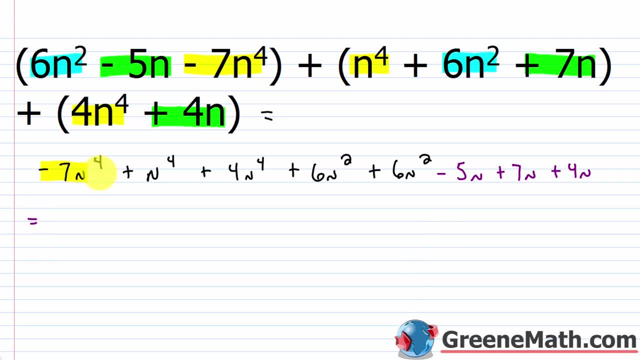 So now we're just going to combine like terms And so I have like terms here. I have- let me do this in a different color- Like terms here, And then I have like terms. I'm going to switch colors again here. So if I look at it, what am I going to have? Negative 7n to the fourth power, plus n to 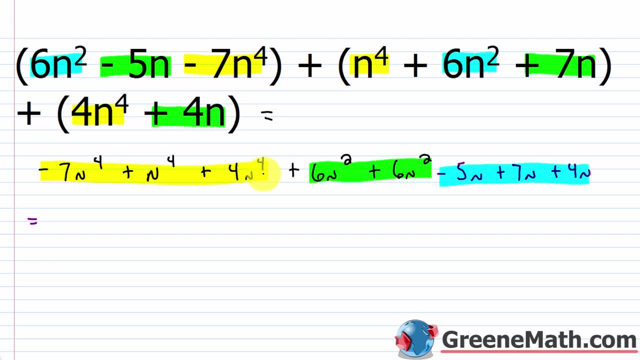 the fourth power plus 4n to the fourth power. Just add the coefficients, So negative 7 plus this coefficient is understood to be 1.. So negative 7 plus 1 is negative 6. Negative 6 plus 4 is negative 2. This would be negative 2 times n to the fourth power, just stays. 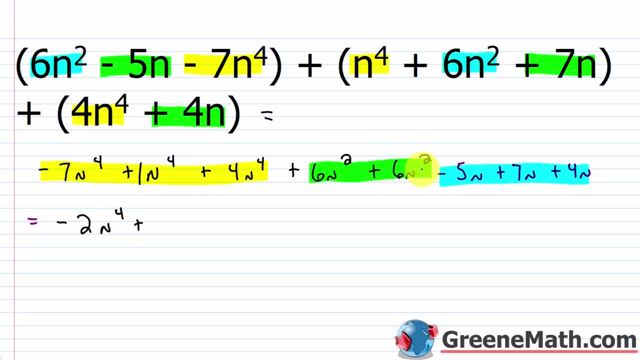 the same. Then plus, You have 6n squared. plus 6n squared, You use 6 plus 6, that's 12 times we have n squared. that stays the same. Then you have negative 5n plus 7n plus 4n, So you have negative. 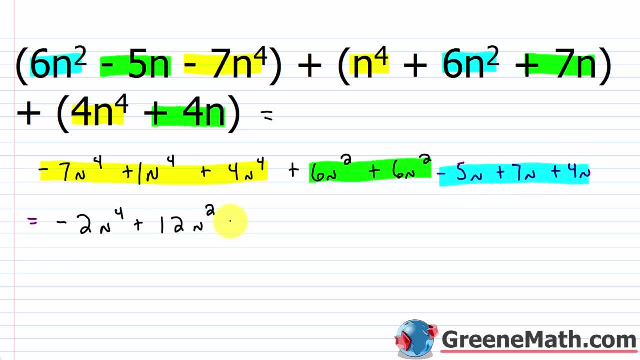 5 plus 7, which is 2, plus 4, which is 6.. So plus 6 times n. So I end up with negative 2n to the fourth power plus 12n, squared plus 6n. All right, now let's get into some subtraction problems. 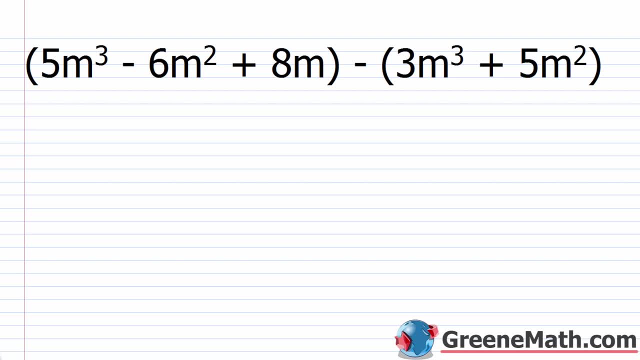 And subtraction is not any more difficult than addition. You just have to know one thing: Whatever polynomial is being subtracted away, what you want to do is you want to change the sign of each term of the polynomial being subtracted away, And then you just add. So 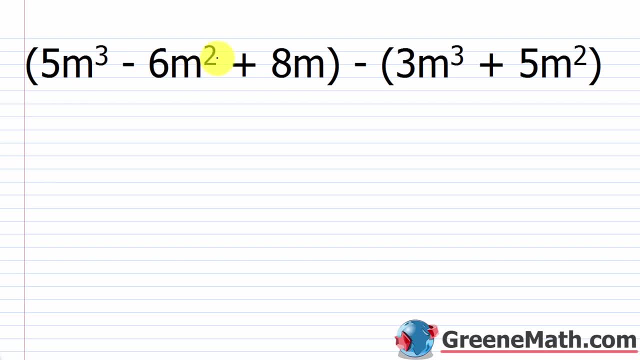 as an example, we have 5m cubed minus 6m squared, plus 8m, Then minus. we have 3m cubed plus 5m squared. Now a lot of students get confused and they're like: well, what's the difference between having this minus 6m squared and minus this whole thing? here The difference. 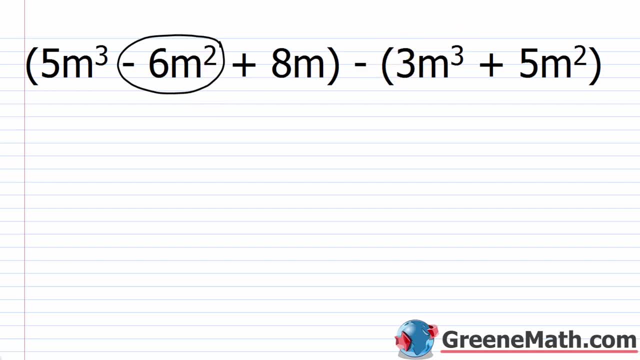 is: I have a minus sign outside of this set of parentheses, So this whole thing is being subtracted away. So if I'm subtracting the whole thing away, what I can do- and you'll see a lot of professors do this- You'll see plus negative. 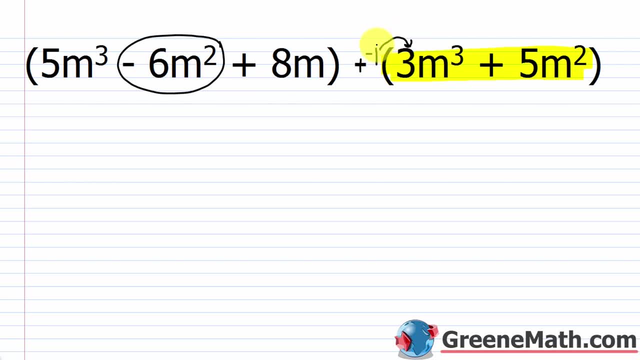 1 there And they'll distribute the negative 1 to each term, just as a reminder to the student to change the sign of each term and then just add. So in other words, if I do it this way, I'd rewrite this problem as 5m cubed minus 6m squared plus 8m Negative 1 times 3m cubed is. 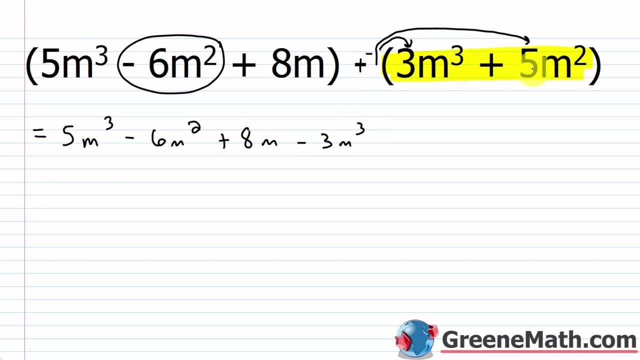 negative 3m cubed And then negative 1 times 5m squared is minus 5m squared. So again, all I'm doing is I'm changing the sign of every term in the polynomial that's being subtracted away. I could have just as easily said: okay, I've got minus 3m cubed and then minus 5m squared. 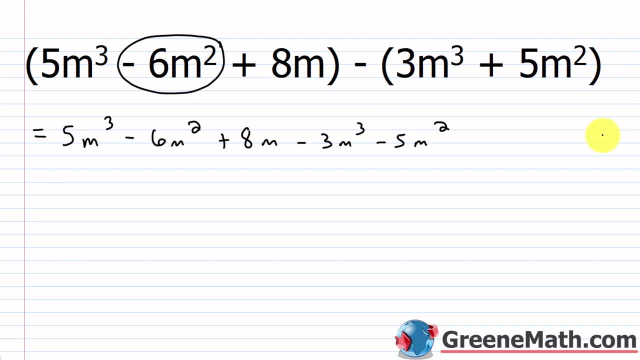 Where students make another mistake is they'll drop the parentheses. They'll say: okay, I have minus 3m cubed. They got the first term right, But then the second term they forget to change. They just leave that as plus 5m squared and they get the wrong answer: You need a minus here and 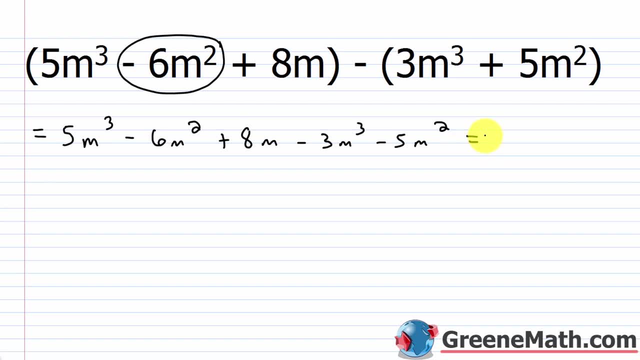 here. Okay, very important. So once you have that, you just combine like terms, like we've been doing with addition. Okay, so it's just one additional step. And to kind of look at this, I would write 5m cubed all the way to the left and then minus 3m cubed. Those are like terms, And then minus. 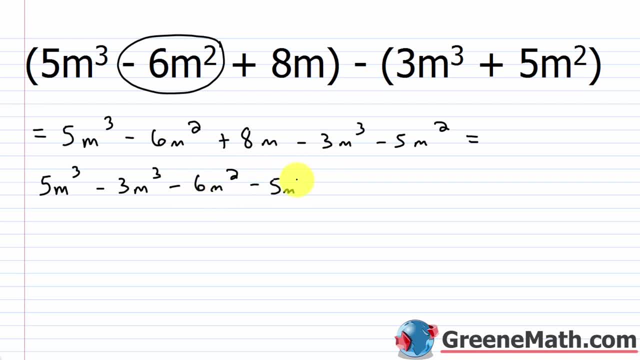 6m squared and then minus 5m squared- Those are like terms- And then plus 8m. So 5m cubed minus 3m cubed is 2m cubed Negative. 6m squared minus 5m squared is negative. 11m squared. And then I have plus 8m. So again, 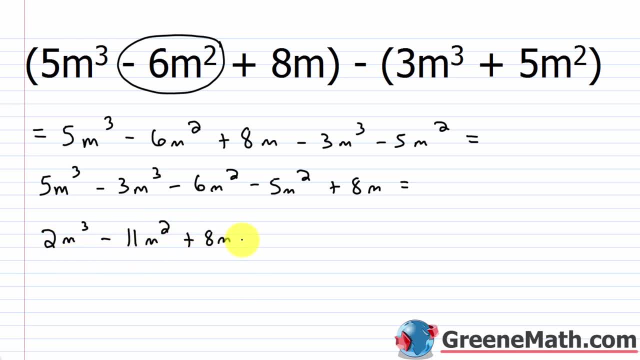 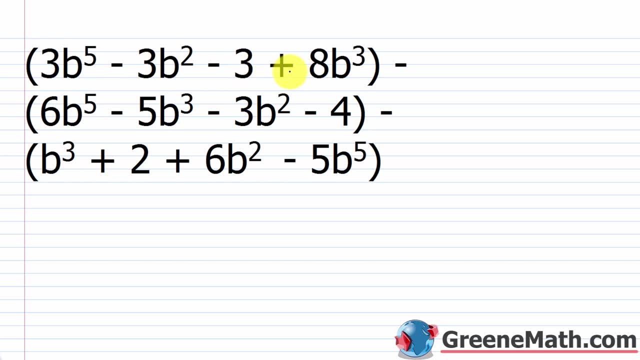 my answer here is 2m cubed minus 11m squared plus 8m. All right, let's take a look at another one. So we have 3b to the fifth power minus 3b squared, minus 3, plus 8b cubed, Then minus. 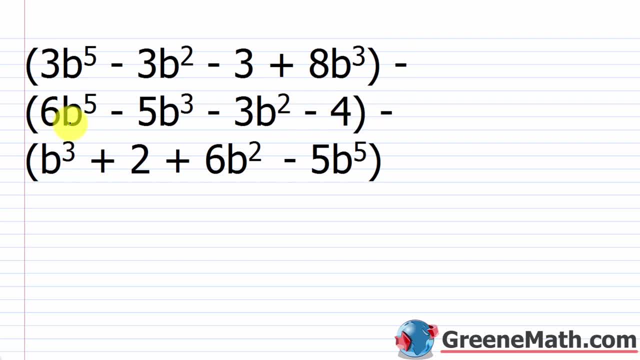 we're subtracting away this whole polynomial here: 6b to the fifth power minus 5b, cubed plus 3b squared minus 4, then minus. I'm subtracting by this whole thing: B cubed plus 2 plus 6, B squared minus 5. B to the fifth power. now the quickest thing you. 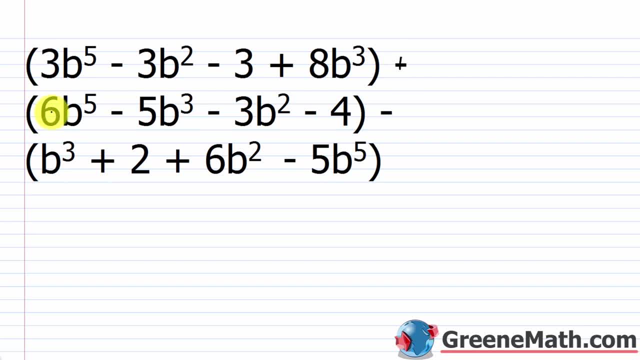 can do again. you can just make this plus and change every sign here. so this would be negative, this would be positive, positive, positive. change the sign here plus negative. this would be negative, negative, positive. okay, change the sign of every term that's being subtracted away. this first polynomial is not being 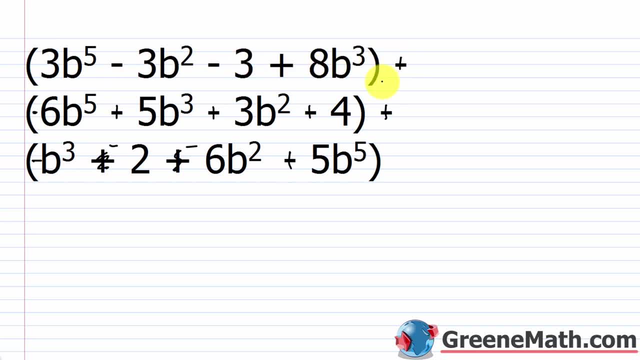 subtracted away. so it just stays as it is. every polynomial that comes after it has a subtraction sign out in front of the parentheses that enclose it. so you've got to put a plus sign and then change every sign for the terms inside of it, the parentheses. okay, very important. you understand that. and again, if you, 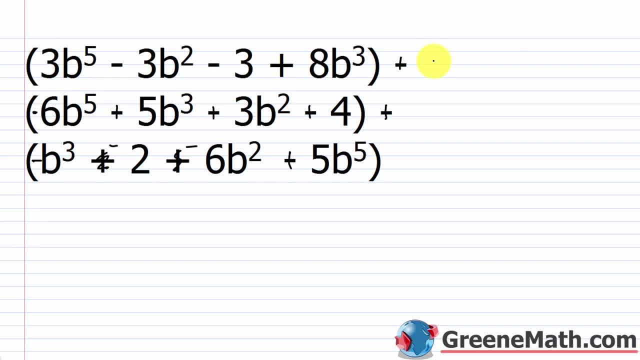 struggle with it. put plus negative 1 and distribute the negative 1 to each term. it's going to remind you to do that. alright, so what I'm gonna do here. if I scan through, I see 5 is the highest exponent. so I've got 3 B to the fifth. 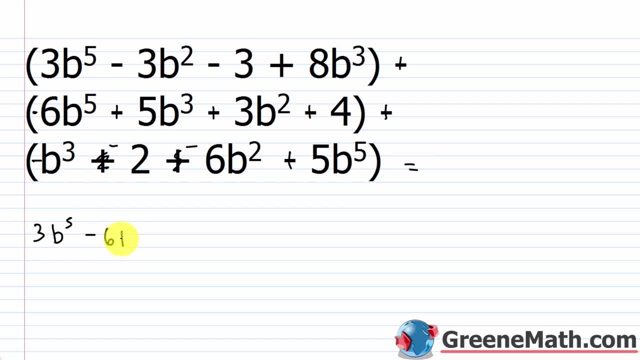 power. I've got negative 6 B to the fifth power and I've got 5 B to the fifth power, so that takes care of this one, this one and this one. all right, so I've got three B to the fifth power, negative 6 B to the fifth power, and that takes care of this one, this one and this one. all right, so I've got. 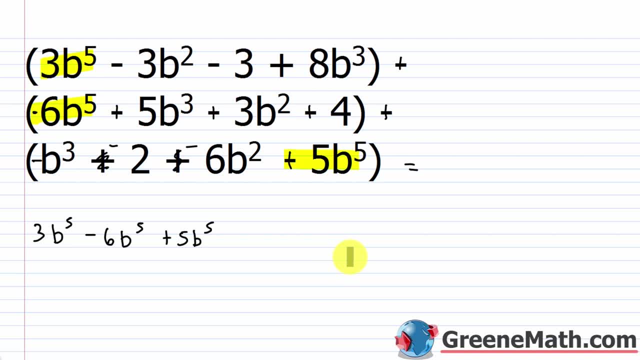 All right, the next highest I see is a three. So I've got 8b cubed, I've got 5b cubed and I've got negative b cubed. okay, So that takes care of this one, this one and this one. 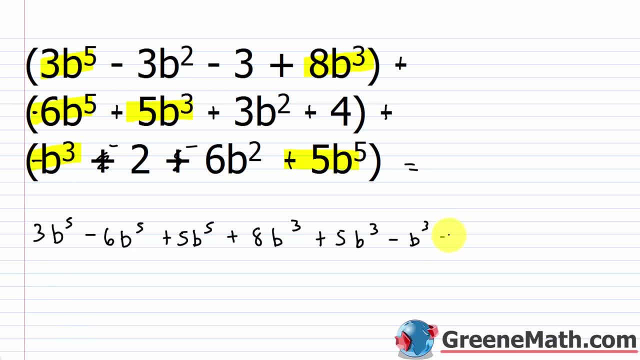 All right, so the next thing I see is b squared, So I've got a negative 3b squared, I've got positive 3b squared and I've got negative 6b squared. So that's gonna take care of this one. 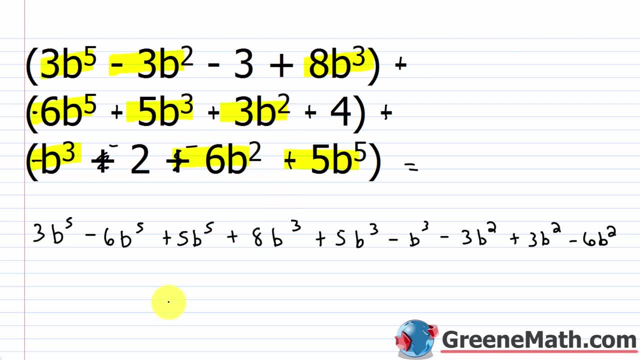 this one and this one, And then, lastly, I have minus three, I have plus four and I have minus two. So that takes care of this one, this one and this one. And because I've highlighted everything, I know I didn't miss anything. 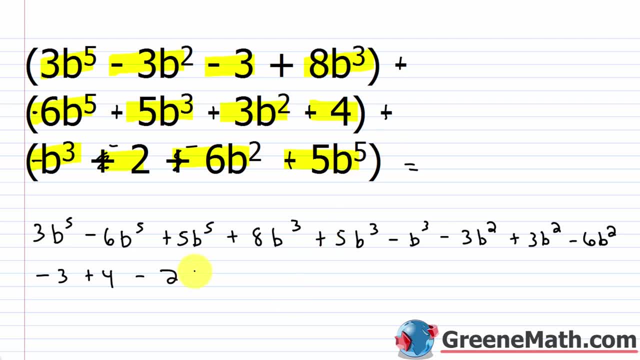 And again it gets very, very tedious with these kind of longer problems. so you need some kind of process to tell you: hey, I've used all of these. So if I start with 3b to the fifth power minus 6b to the fifth power, plus 5b to the fifth power, 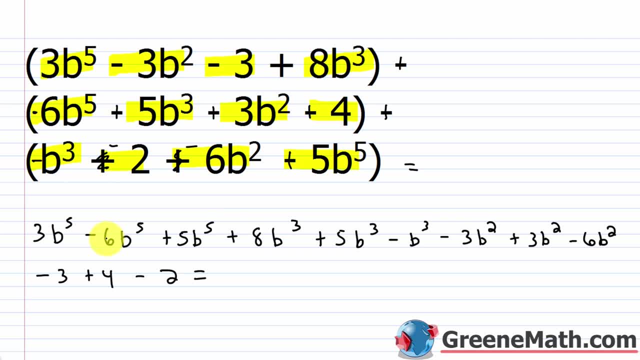 again. look at your coefficients. Three minus six is negative. three plus five is two, So I've got two. and then times b to the fifth power, Here I've got 8b cubed plus 5b cubed, minus b cubed. 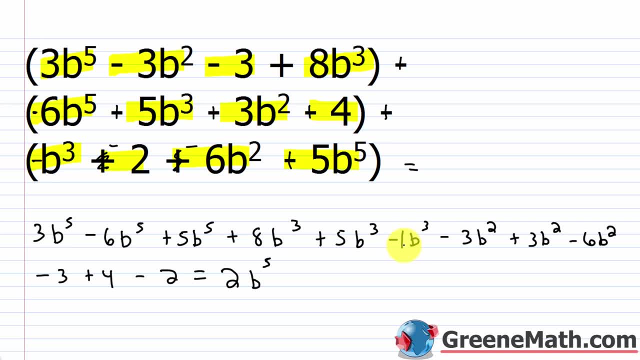 Again, I've got an eight, a five and this would be a negative one. Understand that if you have a variable by itself, the coefficient is one. If you have a negative in front of it, the coefficient is negative one. You can't just not put anything. 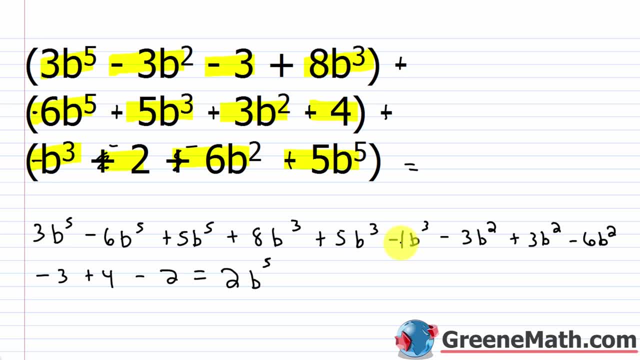 So for this one eight plus five is 13.. 13 minus one is 12.. So this would be plus 12b cubed. Then next I have negative 3b squared plus 3b squared, minus 6b squared. 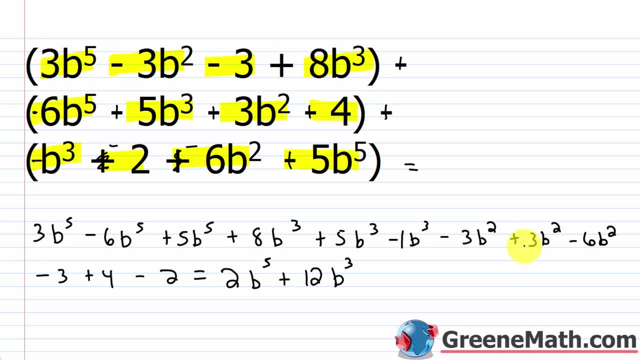 So I think about negative. three plus three is zero, Those are opposites. And then I just have negative 6b squared, So minus 6b squared. And then, lastly, I have negative three plus four, That's one. Then minus two is negative one. 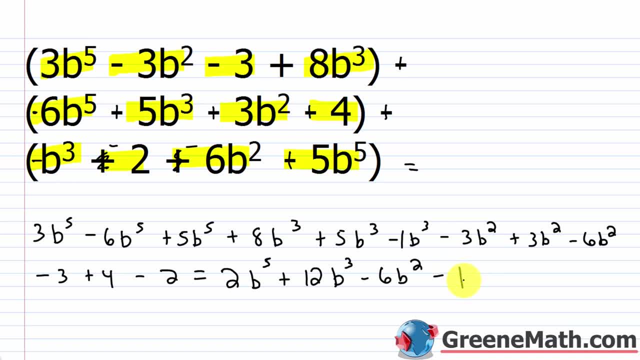 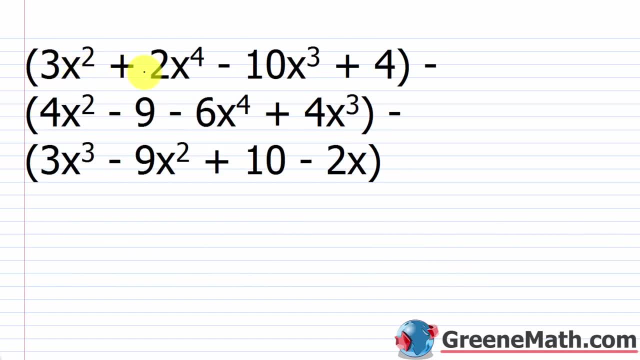 So minus one. So 2b to the fifth power plus 12b cubed minus 6b, squared minus one. All right, the next thing I want to look at is 3x squared plus 2x to the fourth power minus 10x cubed plus four. 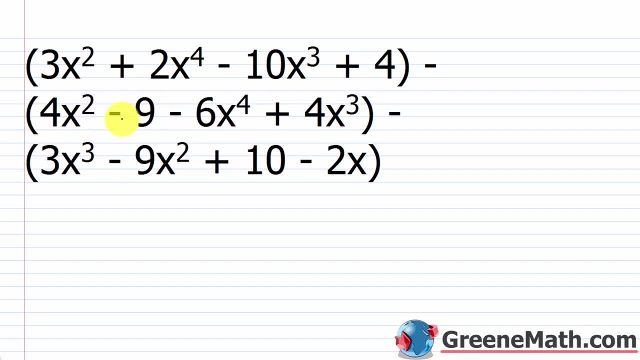 then minus this polynomial, here We have 4x squared minus nine minus 6x squared, So that's the same thing. I have 2x squared minus six x to the fourth power, plus 4x cubed. Then minus, I have 3x cubed minus nine x squared. 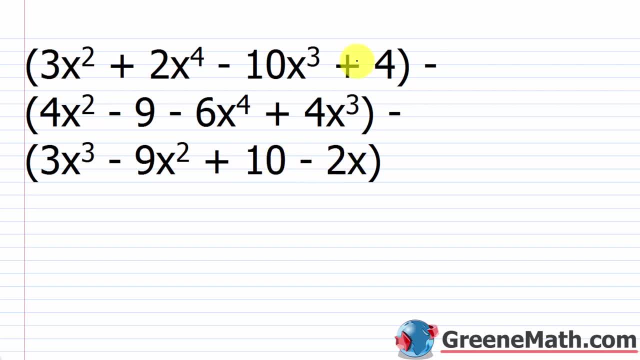 plus 10 minus two x. Again, this first polynomial is just gonna stay the same. So just my 3x squared plus two x to the fourth, power minus 10x cubed plus four. I'm subtracting away this polynomial here. 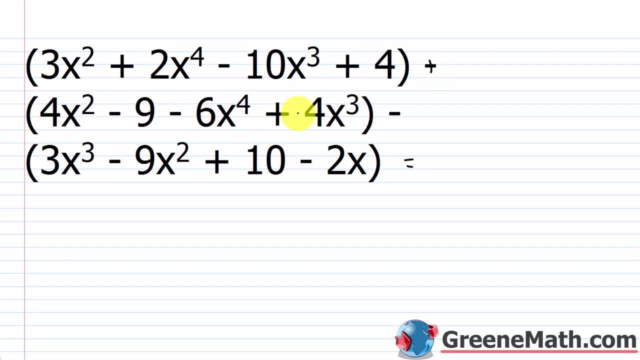 So all I wanna do is put plus and then change the sign of each term So this becomes negative, positive, positive, negative, and then this would be negative For the next one. it's the same. I'm subtracting away this. 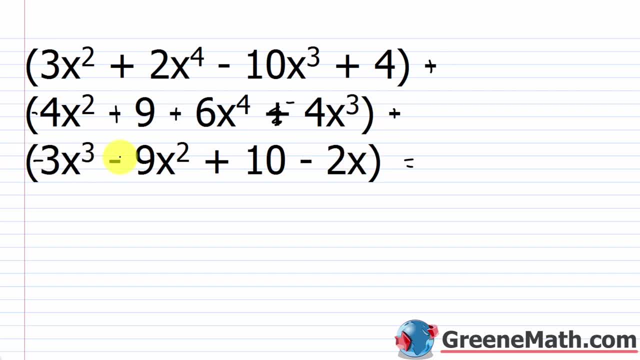 polynomial here. So plus this is negative, positive. you put negative and then positive. All right, So once we've done that, I'm going to scan through. I see four is the highest exponent. So I've got 2x to the fourth power, I've got 6x to the fourth power And I don't have an x to the 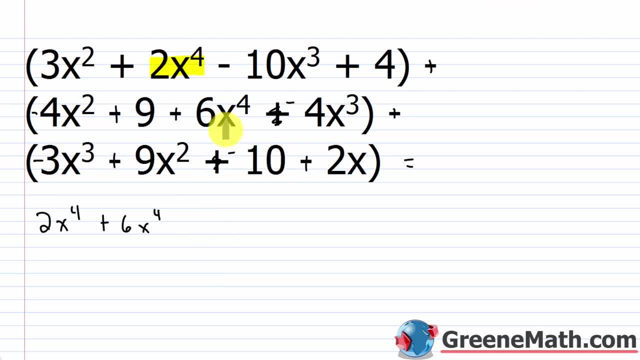 fourth power here. So that just takes care of this and this. Now next I scan through and I see x cubed. So I see I have negative 10x cubed, so minus 10x cubed, And then I have minus 4x cubed. 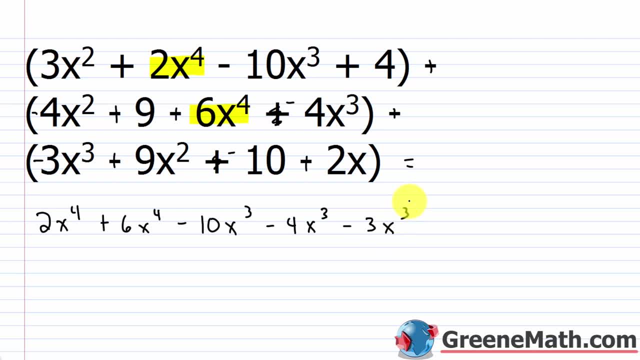 And then I have minus 3x cubed. So that takes care of this, this and this. Then next I see I have x squared, So I have plus 3x squared. I have minus 4x squared And I have plus 9x squared. So that takes care of this, this and 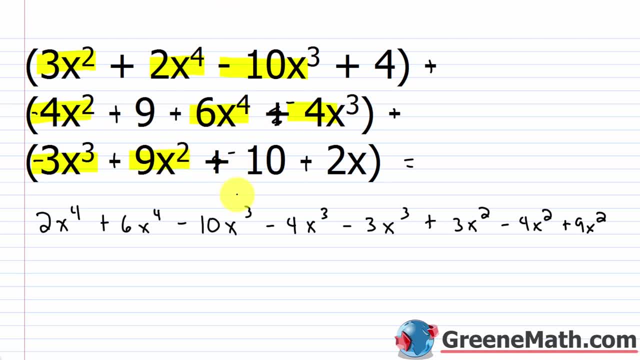 this All right. So, lastly, I have this 2x, So that takes care of this. No more x to the first power anywhere. And then I have 4,, 9, and negative 10.. So plus 4,, plus 9,, plus negative 10, or minus. 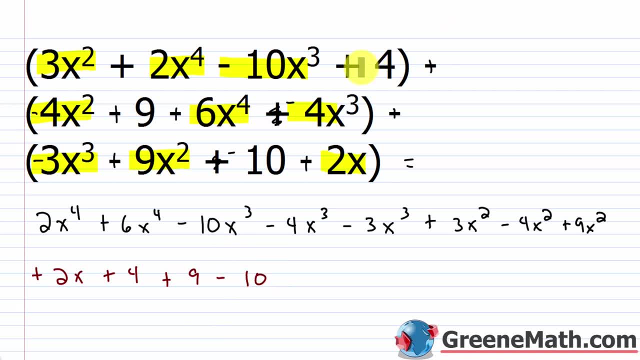 10. Whatever you want to do, All right, So that takes care of this, this and this. And again, notice how I've highlighted everything, so I know I didn't miss anything. OK, So I go through now And I say 2x to the fourth. 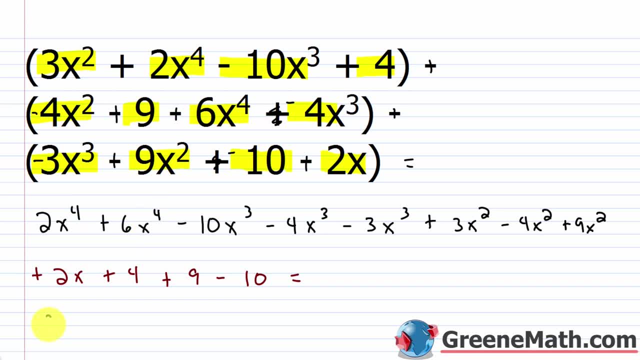 power plus 6x to the fourth power. 2 plus 6 is 8 times x to the fourth power. Then next I have minus 10x cubed, minus 4x cubed, minus 3x cubed, So I've got negative 10 minus 4.. That's negative. 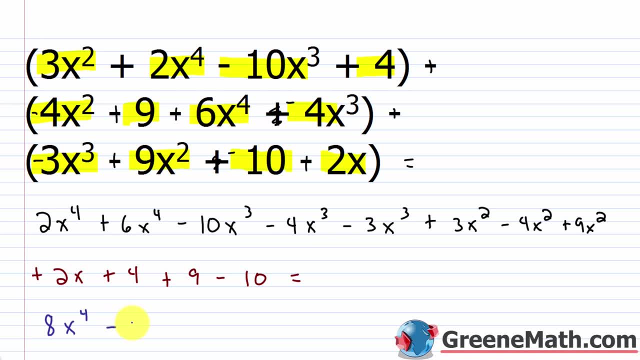 14. Minus 3. That's negative 17. So I've got negative 10 minus 4.. That's negative 14.. That's negative 17. So minus 17,. then times x cubed, Then I continue. I have 3x squared minus 4x. 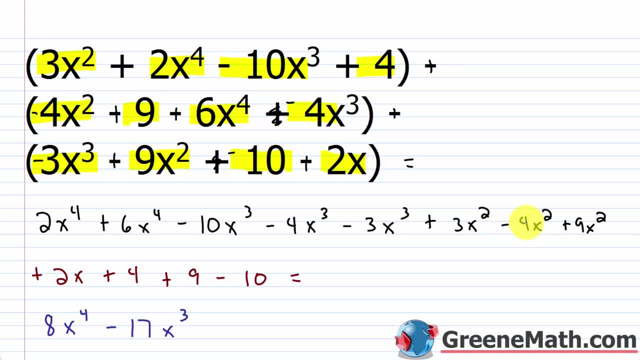 squared, plus 9x squared, So I've got 3 minus 4. That's negative 1. Plus 9 is going to give me 8. So this is plus 8x squared. Then I have my plus 2x- Nothing to combine with that, And then I have 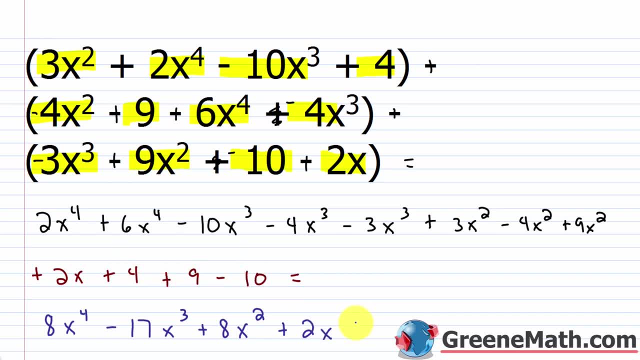 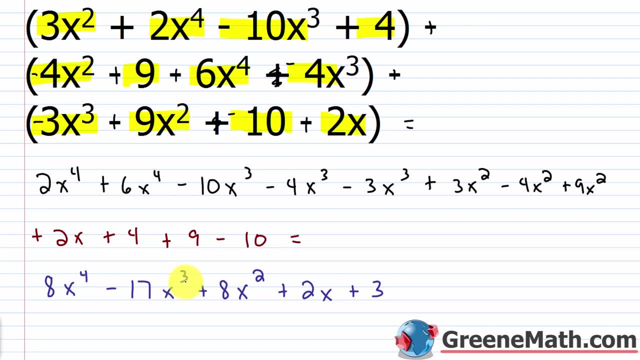 4 plus 9,, which is 13,, minus 10,, which is 3.. So plus 3.. So we end up with 8x to the fourth minus 17x cubed, plus 8x squared, plus 2x plus 3.. 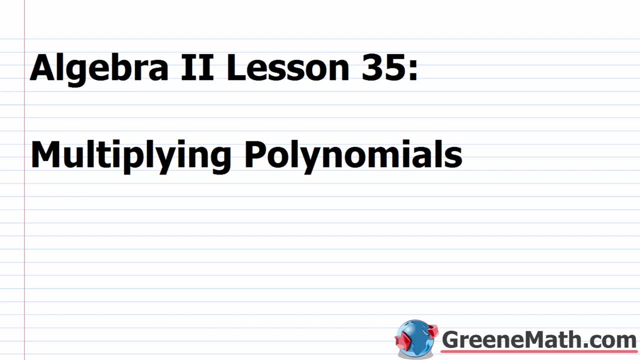 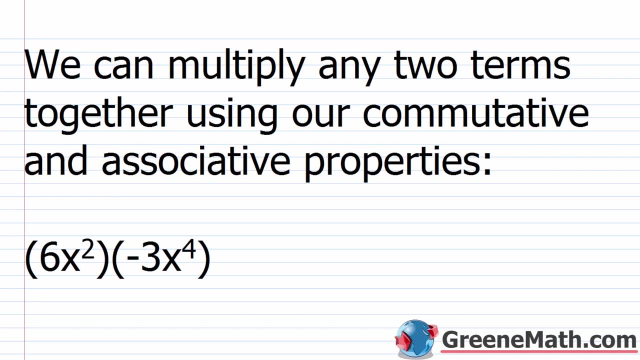 Hello and welcome to Algebra 2, Lesson 35.. In this video, we're going to learn about multiplying polynomials. So, as I've said in a lot of videos in Algebra 2, most of you will find multiplying polynomials as just a review. We learned this back in Algebra 1. And it's really 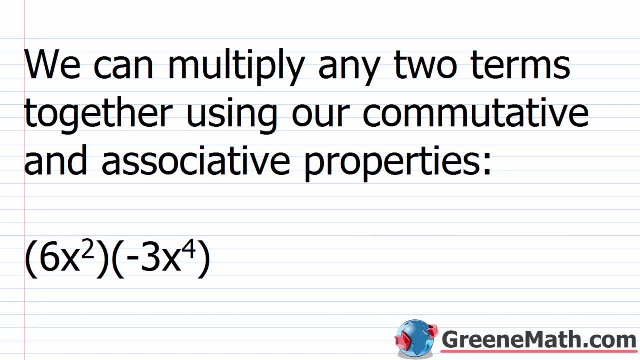 quite an easy process. So I'm going to start at the very beginning with just multiplying two monomials together. right, Two single term polynomials together. So I have here that we can multiply any two terms together using our commutative and associative properties. Remember. 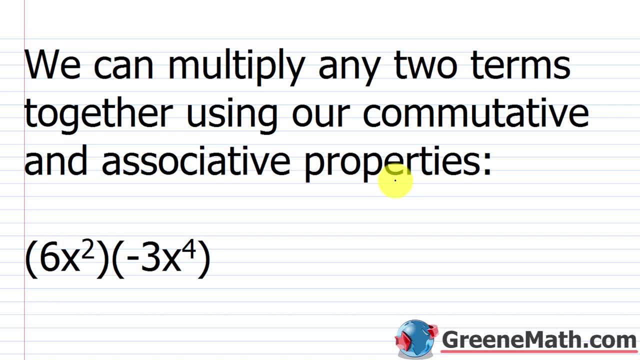 the commutative property tells us we can multiply in any order And the associative property tells us that the grouping doesn't matter when we multiply. So, in other words, if I look at 6x squared times negative 3x to the fourth power, what I can do is I can rearrange things. 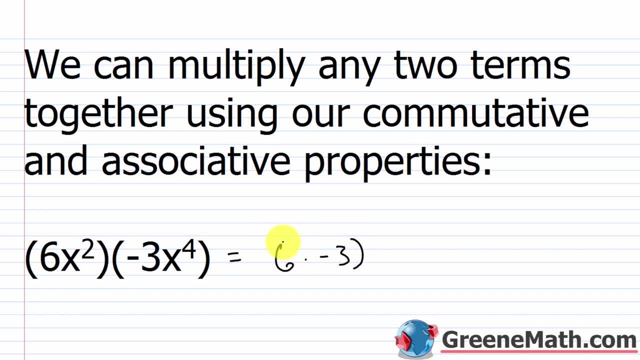 So where I put the 6 next to the negative 3, and I could group those together And then I could multiply this by the x squared times the x to the fourth power. Now, once I do this, I make it completely obvious how to find the answer here. I know that 6 times negative 3 is negative 18.. 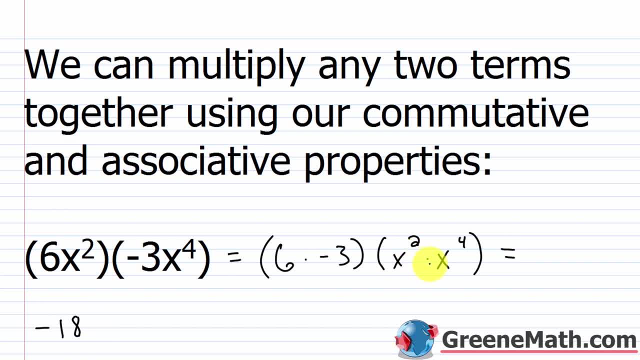 I can just write that out in front. And I know that x squared times x to the fourth power from the rules of exponents x stays the same. I would add, the exponents 2 plus 4 is 6.. So the answer here is negative. 18x to the sixth power. 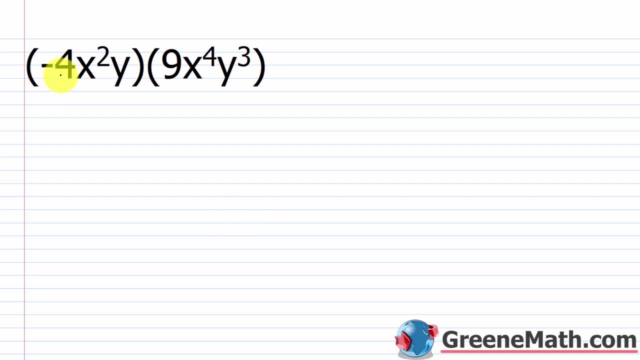 All right, let's take a look at another one just like that. So we have negative 4x squared y. This is multiplied by 9x to the fourth power, y cubed. So again I can just rearrange things to make it easy to see what I need to do. Let's put the coefficients in one group. So let's say: 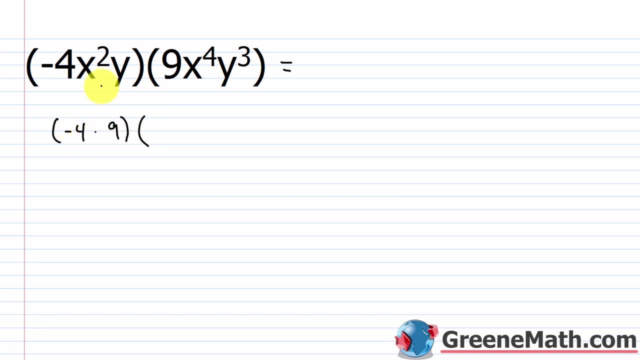 we have negative 4 multiplied by 9.. And then another group: let's do the x variable, So x squared times x to the fourth power. And then in another group let's do y, So we have y times y cubed. So again we set it up like this. We make it completely obvious what we need to do. 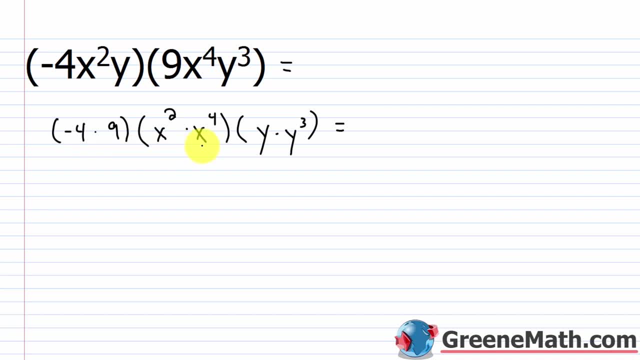 And once we kind of get rolling with this- we're not going to take the time to break it down this way- We'll be able to mentally multiply two terms together and write our answer. But for now we do negative 4 times 9.. That's negative 36.. We have x squared times x to the fourth power, That's x. raised to the power of 2 plus 4, which is 6.. And then we have x squared times x to the fourth power. And then we have x squared times x to the fourth power, That's x raised to the power of 2 plus 4, which is 6.. 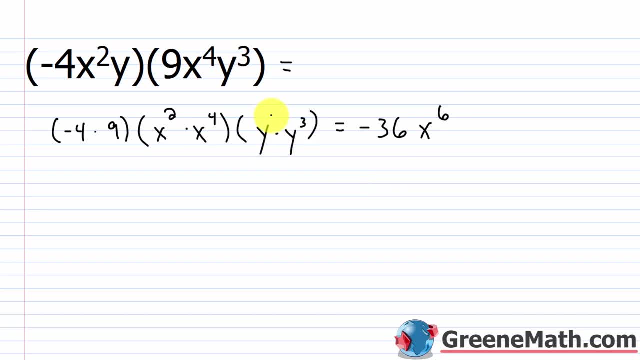 Then we have y times y cubed, Remember. this exponent is understood to be 1.. So the base y stays the same. The exponent 1 plus the exponent 3 gives me an exponent of 4.. So my answer here is negative. 36x to the sixth power, y to the fourth power. All right, so let's kind of move. 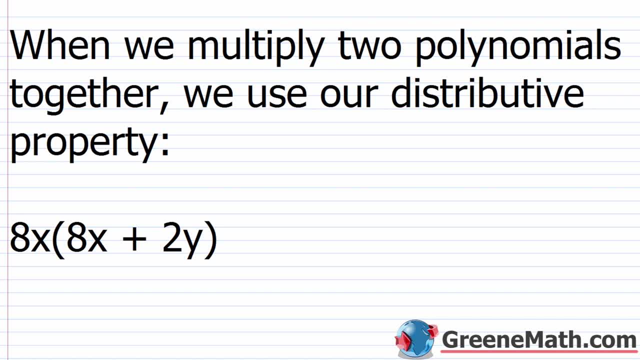 on now. So when we multiply two polynomials together, we're basically using our distributive property. So if I have a polynomial 8x, so this is my distributive property, And then I have a polynomial 8x plus 2y. This is just a monomial, It's a one-term polynomial And I multiply by this. 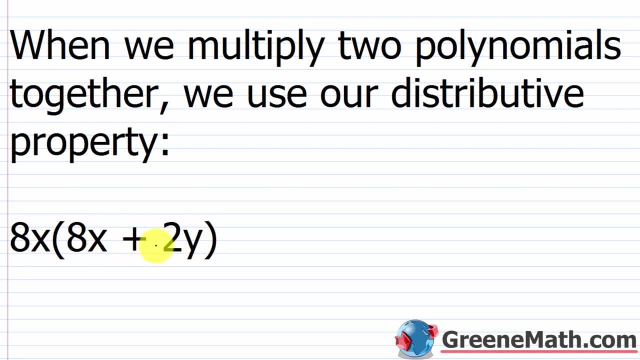 binomial that's, inside of parentheses, 8x plus 2y. What would I do? Well, again, I have something outside of parentheses, So we just use our distributive property. So I'd multiply 8x times 8x, So 8x times 8x. Then, plus, we'd have 8x multiplied by 2y. So 8x times 2y, And again. 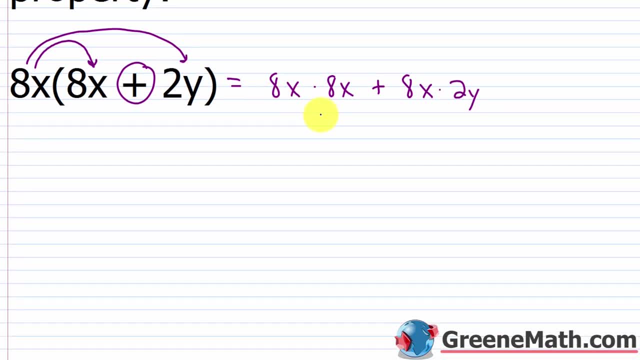 as I just told you, we're not going to take the time to kind of regroup things every time. We know that if I'm multiplying 8x times 8x, the first thing I'm going to do is multiply the coefficients together. 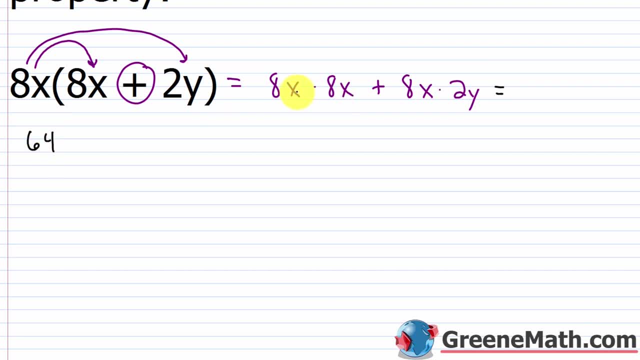 8 times 8 would be 64. Then next I'd multiply my variables. I have x times x. Again, this is an understood exponent of 1.. This is an understood exponent of 1.. So x stays the same. We add 1 plus. 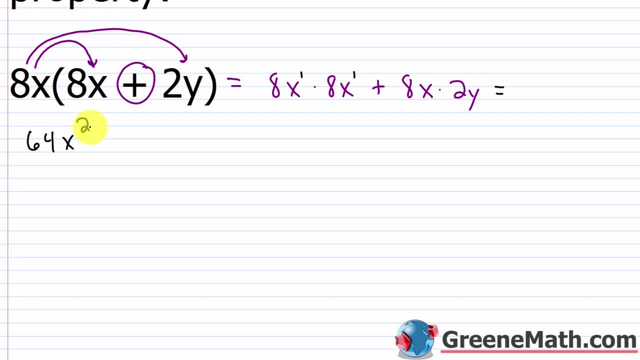 1, and we get 2.. So that's 64x squared. Then plus, Now I have 8x times 8x. So 8x times 8x, And again, this is an understood exponent of 1.. This is an understood exponent of 1.. So 8x times 8x, So 8x times. 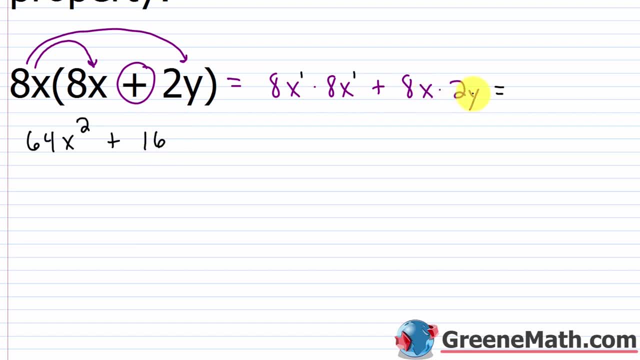 2y. 8 times 2 is 16.. x times y is what. Those aren't the same variable, so it's just xy. Now, because these are not like terms, I cannot simplify this any further. Okay, So I leave the answer as: 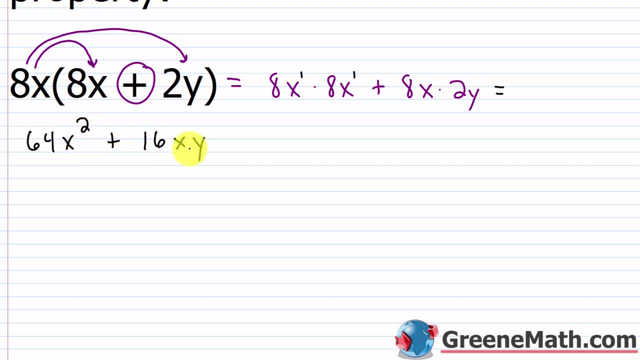 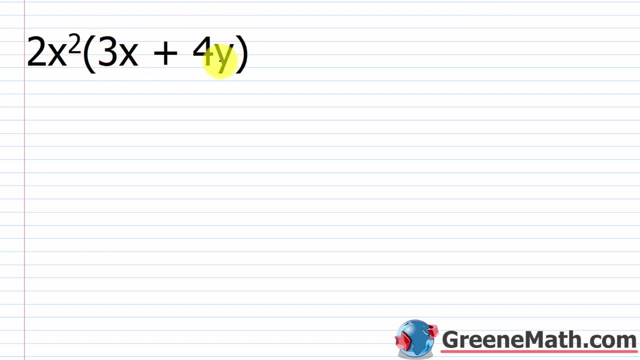 64x squared plus 16xy. All right, let's take a look at another one. So if we had 2x squared times the quantity 3x plus 4y, Again you've got a monomial times a binomial. 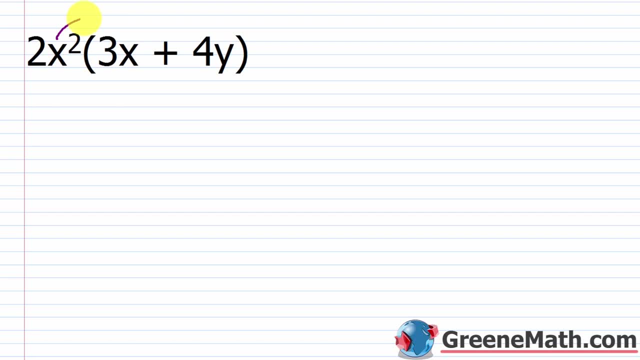 So I'm going to take this guy right here, this 2x squared, and I'm going to distribute it to each term inside of the parentheses. So I would have 2x squared times 3x, then plus 2x squared times 4y. 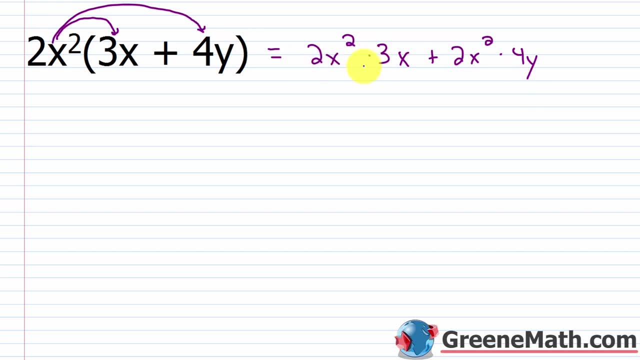 So in this first part right here, 2 times 3 would be 6, and then x squared times x would be x. cubed Again, you've got to understand that this exponent is 1.. Then we'd have plus. We'd have 2x squared times 4y. 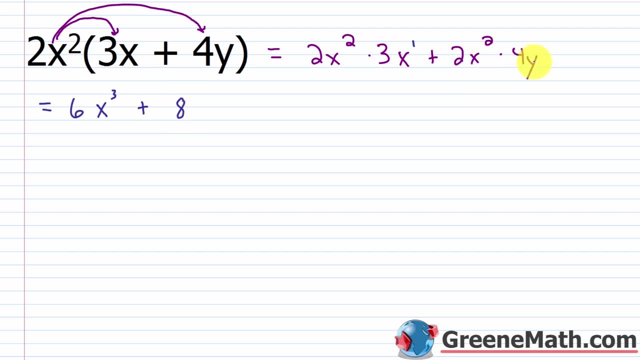 So 2 times 4 is 8, and then x squared times y. all I can really do there is write x squared y. So this is 6x cubed plus 8x squared y. Alright, so now we come to another section. 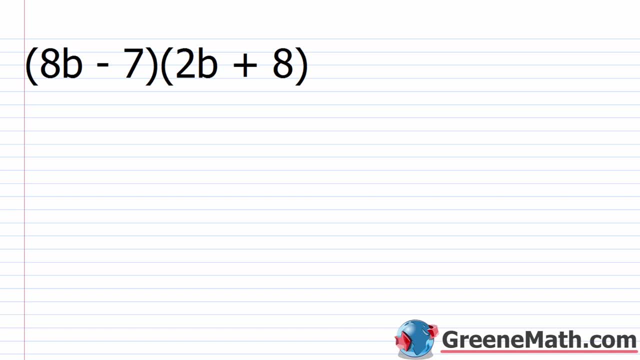 We're going to multiply two binomials together, And most of you again who have taken Algebra 1, know that we can use something called FOIL- Okay, FOIL- to do this, But I'm not going to use FOIL just yet. We'll get to that at the later part in the lesson. 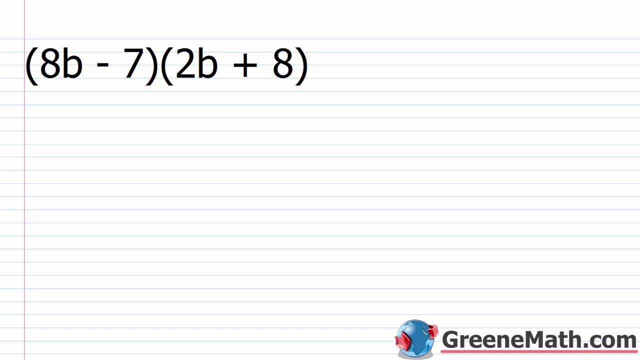 I'm going to show you a different way to do this. So we'll use our distributive property, And what we basically want to think about is each term of the first polynomial is going to be multiplied by each term of the second polynomial. So, in other words, I would take 8b, the first term of the first polynomial, and multiply it by the second polynomial. 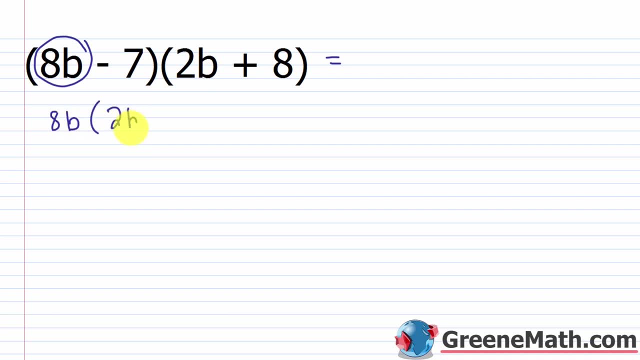 So we would have 8b multiplied by the quantity 2b plus 8b. Then I'm going to add to that, I'm going to take this second term of the first polynomial and I'm going to do the same thing. 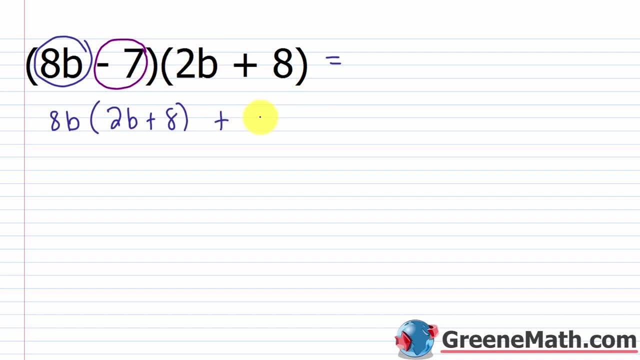 I'm going to multiply it by each term of the second polynomial. So plus we'd have negative 7, multiplied by the quantity 2b plus 8.. So again I'm going to use my distributive property: 8b times 2b would be 16b squared. 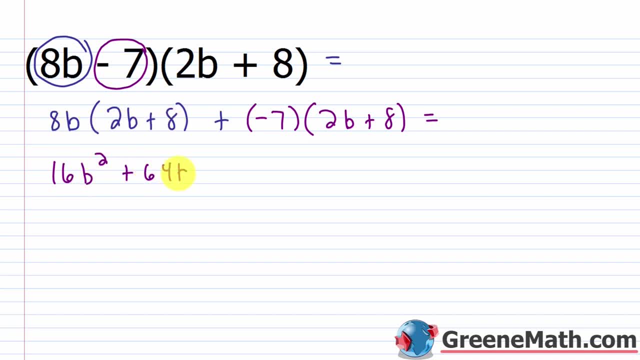 8b times 8 would be 64b. Then plus You have negative 7 times 2b, That's negative 14b. Then you have negative 7 times 8, which would be negative 56. Now, in this particular case, we do have like terms. 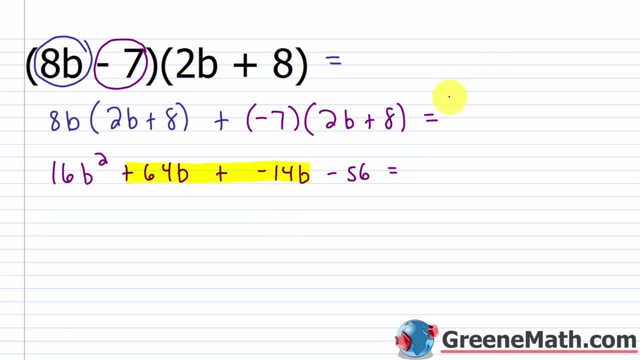 The two terms in the middle here can be combined because they have a common b to the first power. So I'm going to rewrite 16b squared. That's not going to change. 64b plus negative 14b would be 50b. 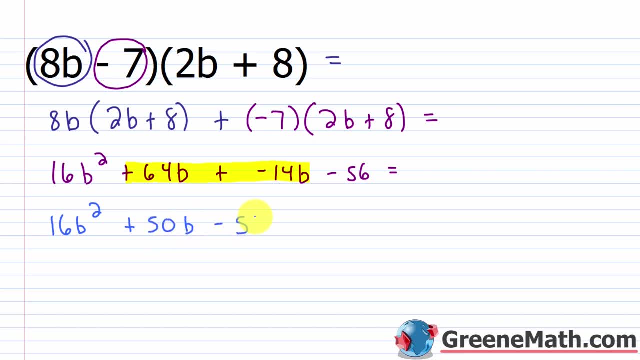 So plus 50b And then minus 56. Now I don't have any more like terms. so that's my answer: 16b squared plus 50b, minus 56.. All right, Let's take a look at another one like that: 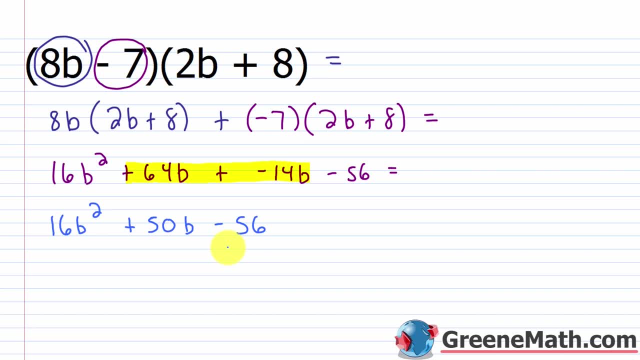 Again we have the product of two binomials. And again, if you wanted to use FOIL at this point, you could. If you know it, you could use it. But I want to do it again a different way. So I'm going to take each term of the first polynomial, multiply by each term of the 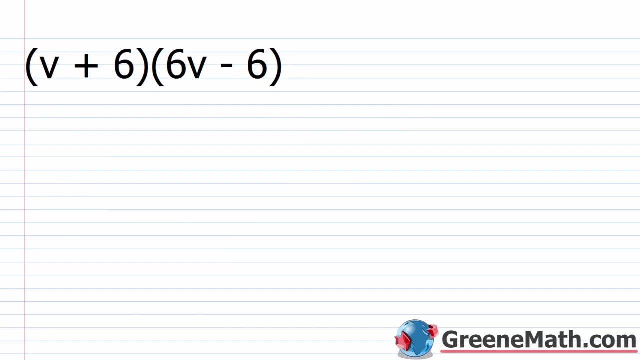 second. So I'm going to start out with v And then I'm going to multiply it by the second. So I'm going to take each term of the first polynomial, multiply by each term of the second. So I'm going to start out with v. 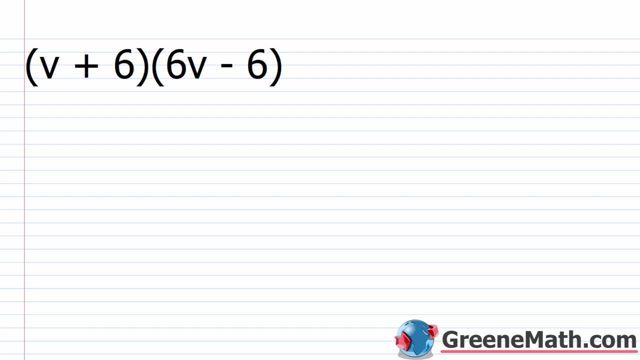 And then I'm going to multiply by the second. And again, if you wanted to use FOIL at this point, you could. If you know it, you could use it, But I want to do it again a different way. So I'm going to take each term of the first polynomial, multiply by each term of the second. 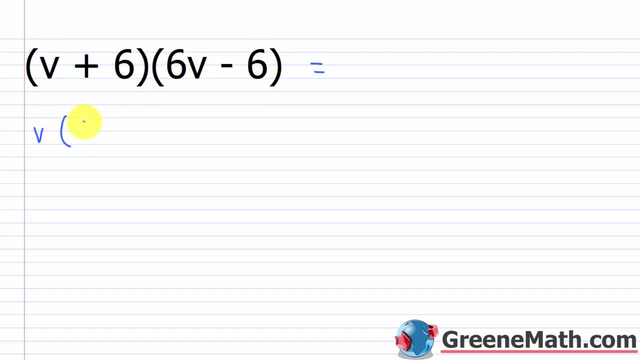 So I'm going to start out with v being multiplied by the quantity 6v minus 6.. And then I'm going to add to that 6 multiplied by the quantity 6v minus 6.. And again, using FOIL is just a way to keep track of things. 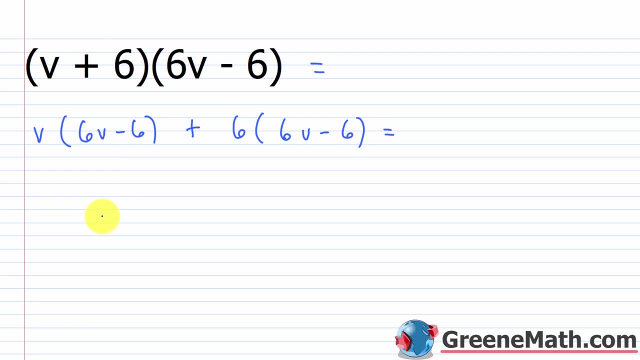 It's a way to remember or easily accomplish things. Okay, So that's how you accomplish the same task. So v times 6v would be 6v. squared v times negative 6 would be minus 6v. Then you'd have plus 6 times 6v is 36v. 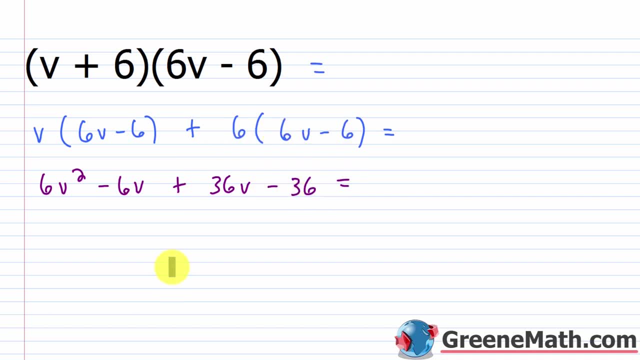 And then 6 times negative, 6 would be minus 36.. Again, you have like terms in the middle here, So I'm going to rewrite 6v squared. So 6v squared Negative, 6v plus 36v is plus 30v. 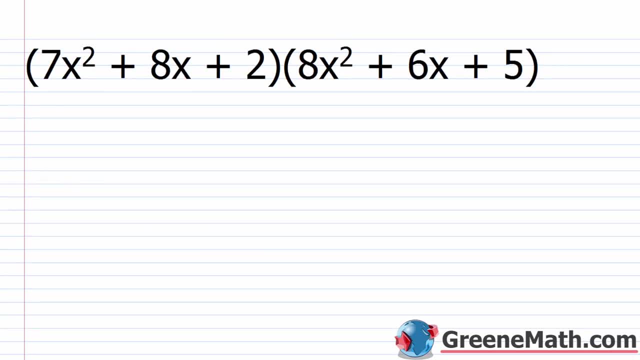 and then minus 36.. All right, so let's talk about one that's a little bit more tedious. What if you get a trinomial times a trinomial? As we get more terms involved in the multiplication, it becomes much more tedious. 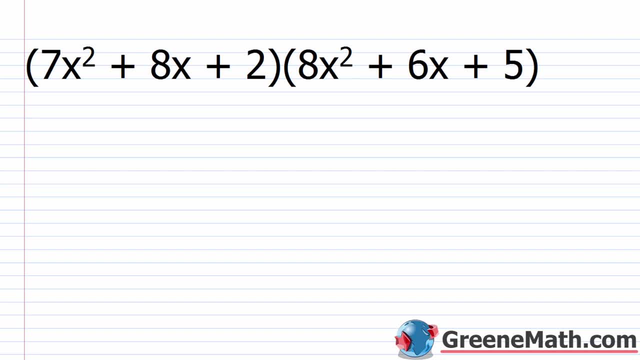 Not any harder. The operation is the same. It's just more tedious, more things to keep track of. So we don't have anything like FOIL for this. What we have to do is we have to take again each term from the first polynomial. 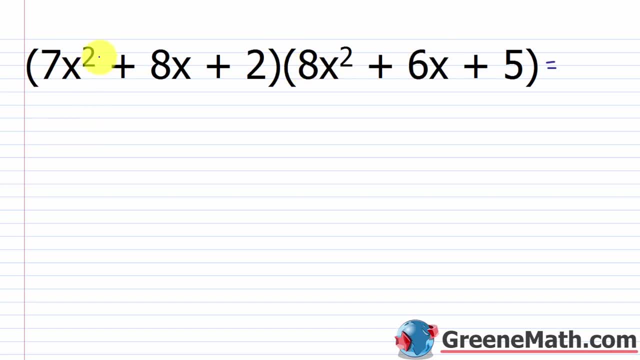 multiply it by each term of the second polynomial. So in other words, I'd start out with 7x squared and that's going to be multiplied by this guy right here, this 8x squared plus 6x plus 5.. 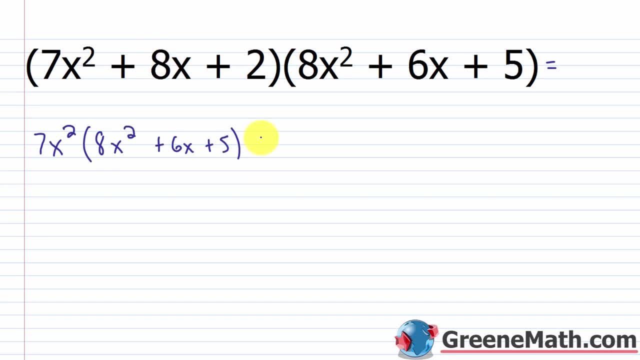 Then I move to the next term in the first polynomial. So I have plus this guy right here. So 8x multiplied again by this second polynomial, 8x squared plus 6x plus 5. Then we'd have plus 2.. 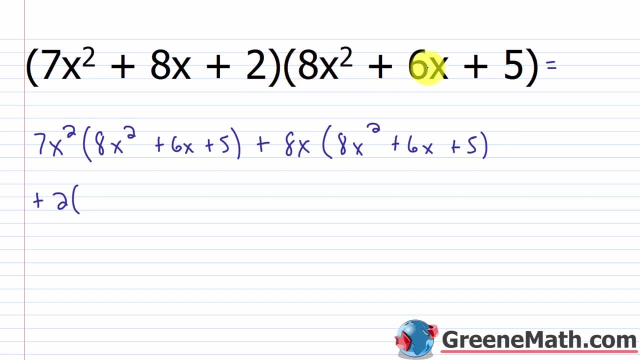 That's the final term of the first polynomial and that's going to be multiplied by the second polynomial. So times 8x squared plus 6x plus 5, and this equals. So now I'm just going to go through and use again. 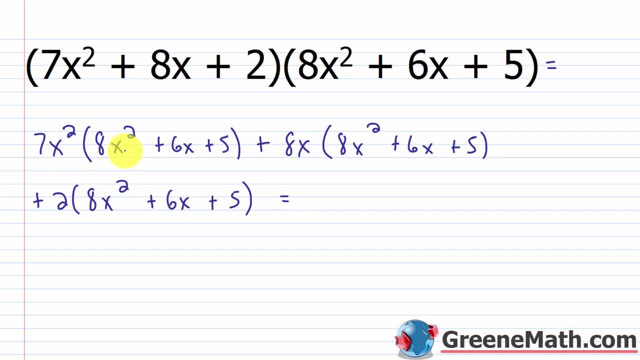 my distributive property everywhere. So 7x squared times 8x squared would be what? Well, we've got to think about. 7 times 8 is 56. We know that x squared times x squared is x to the fourth polynomial. 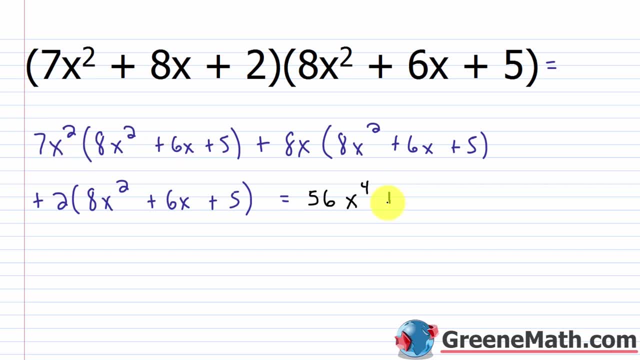 7x squared times 6x. 7 times 6 is 42, and then x squared times x is x cubed. Then we have 7x squared times 5.. So we know that 7 times 5 is 35,. 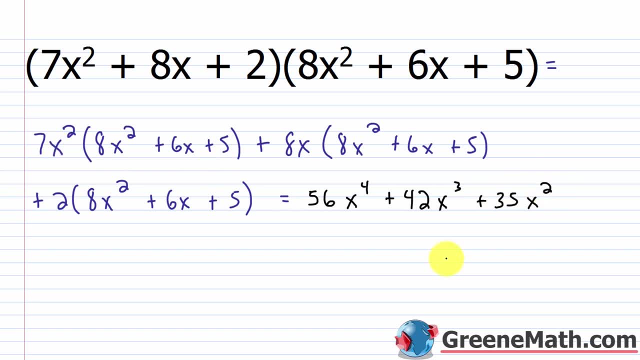 and then x squared would come along for the ride. All right, So let's move down to this one now. So 8x times 8x squared would be what? 8 times 8 is 64.. x times x squared is x cubed. 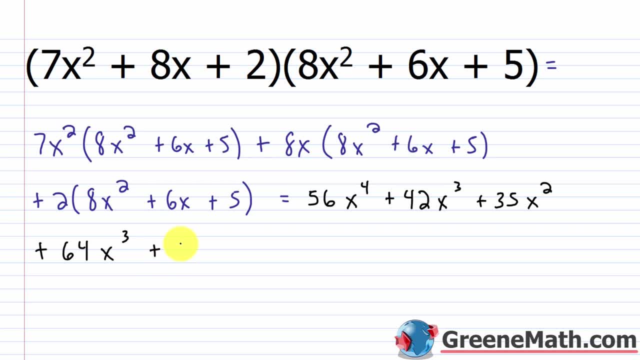 Then 8x times 6x would be what. You know that 8 times 6 is 48.. x times x is x squared. Then we have 8x times 5.. We know that 8 times 5 is 48.. 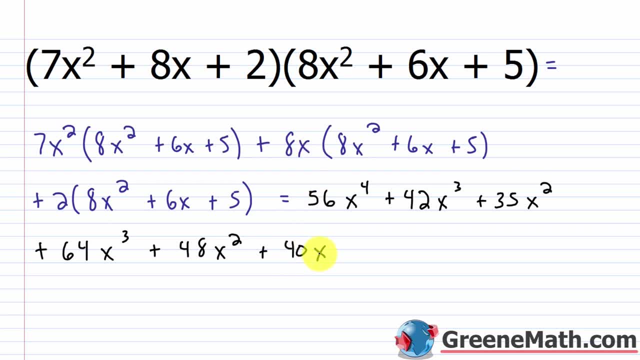 So plus 40, and x comes along for the ride. All right, We've got one more of these to do. So now we've got 2 times 8x squared, That's 16x squared. Then 2 times 6x, that's going to be 12x. 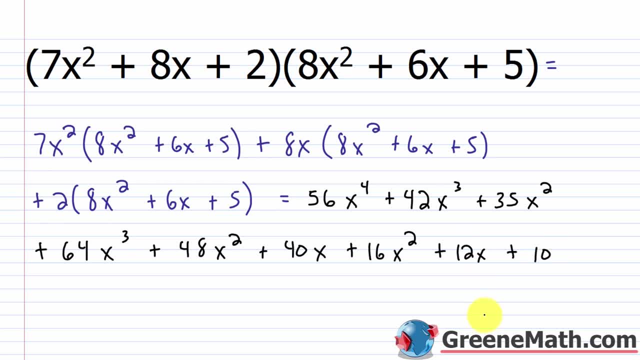 And then 2 times 5 would be 10.. So all that work. We're still not done, though, because we have to combine like terms. If you look, we have what We have: 56x to the fourth power. 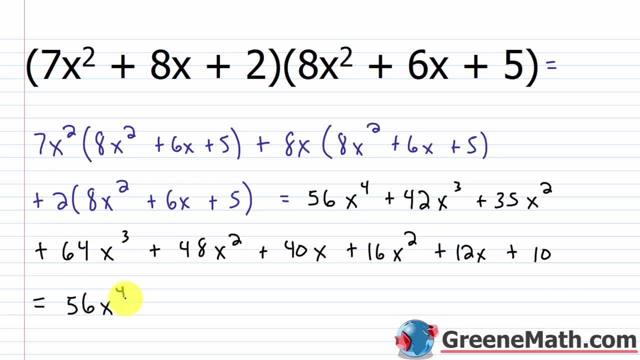 nothing to combine with that. But if I look at 42x cubed, I've got like terms here, So I've got 42x cubed and 64x cubed So we can combine those into 106, because 42 plus 64 is 106,. 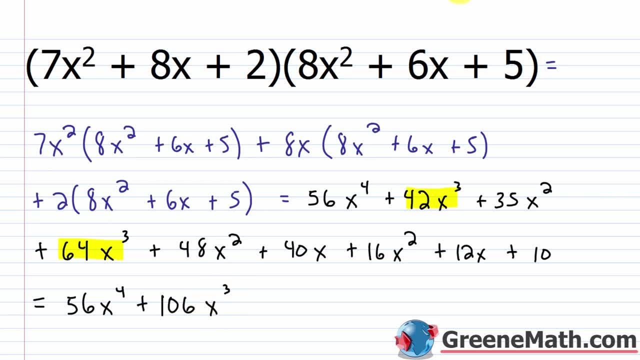 and then x cubed. Now the next thing I'm looking at is x squared. I've got 35x squared here, I've got 48x squared here And I've got 16x squared. So if I add 35,, 48, and 16,, I would get 99.. 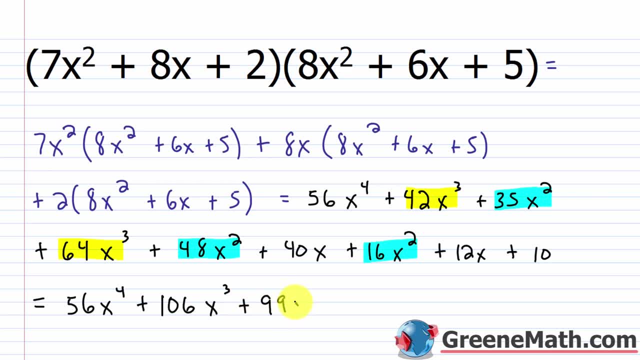 So next I'd have plus 99x squared- And let me make that 2 a little bit better- And then I have x to the first power. I've got 40x here. I've got 12x here. So 40 plus 12, we know, is 52.. 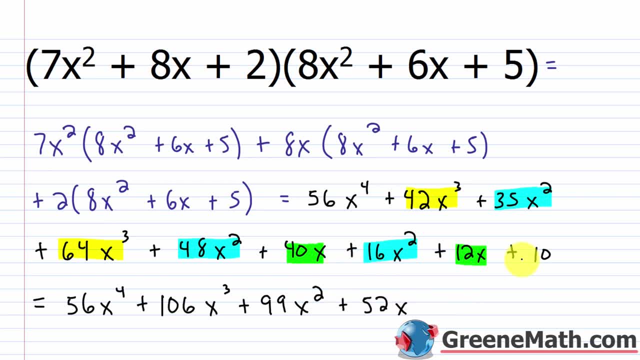 So this would be plus 52 and then x, And lastly you just have plus 10.. So plus 10,, nothing to combine. So you can see how tedious a problem like this is. It just takes a lot of time to just set it up. 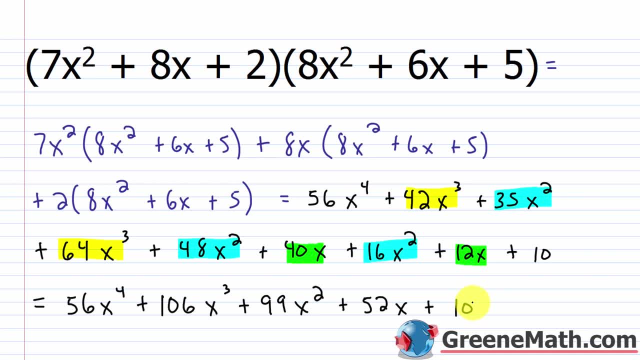 get going, combine like terms, And the more terms you have involved, the easier it is just to make a mistake. So you want to just be very, very careful when you're working. problems with a lot of terms. All right, let's take a look at one more like this: 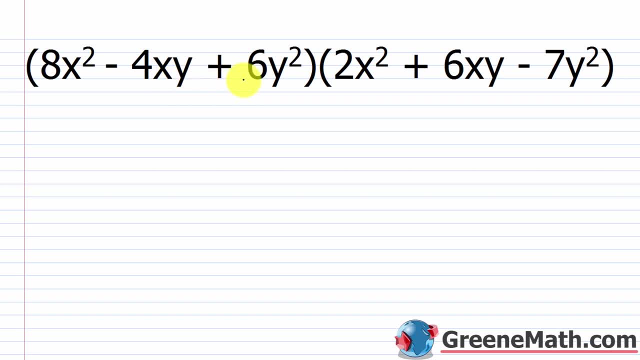 So if I had the quantity 8x squared minus 4xy plus 6y squared and I multiply this by the quantity 2x squared plus 6xy minus 7y squared again, what I want to do is take each term. 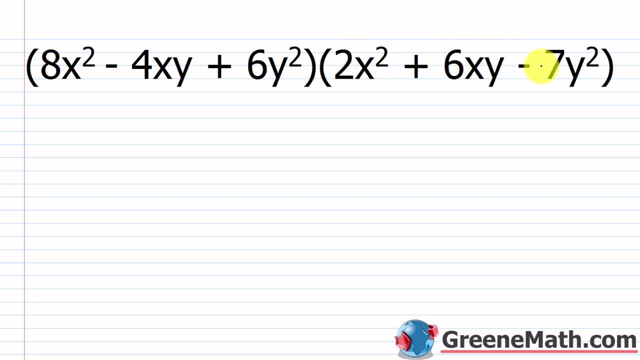 from the first polynomial multiplied by each term of the second polynomial. Now you don't have to go through and set it up like I did the last time. You can do this more mentally. So I could start out with this term right here. 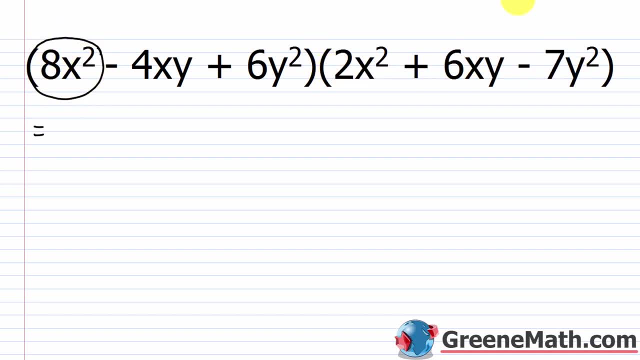 8x squared, multiplied by this polynomial here. Let me just highlight this real quick so we know what we're working with. So this times this: okay. So 8x squared times 2x squared, 8 times 2, is 16.. 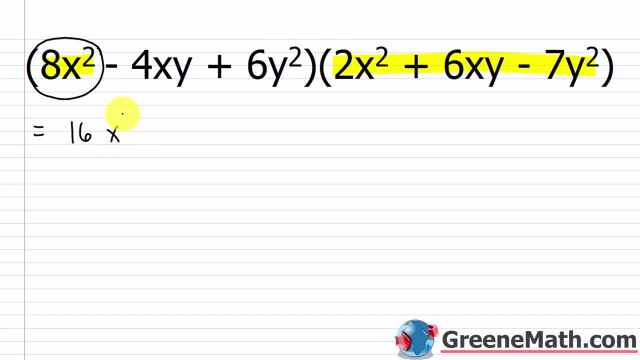 X squared times x squared is x to the fourth power. Then next let's say 8x squared times 6xy. So 8 times 6 is 48. Then we'd have x squared times xy. Now, x squared times x would be x- cubed. 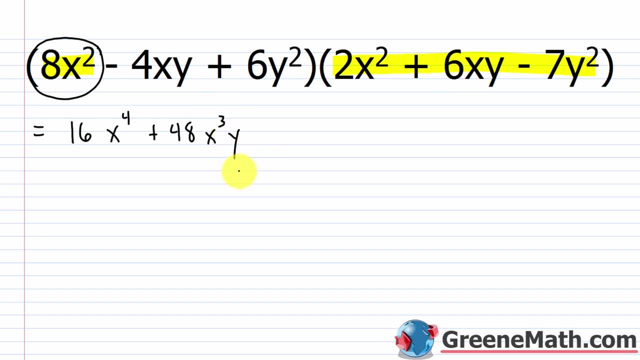 and then y would just come along for the ride. Now, lastly, I'd do 8x squared times negative: 7y squared 8 times negative: 7 is negative 56.. And then x squared times y squared would be x squared. 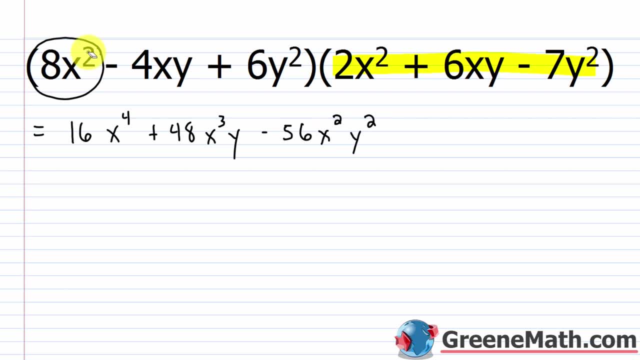 and then y squared would be x to the fourth power. Okay, so good to go there. So let me erase this. We're moving down to this term right here, this negative 4xy. So if I did negative 4xy times 2x squared. 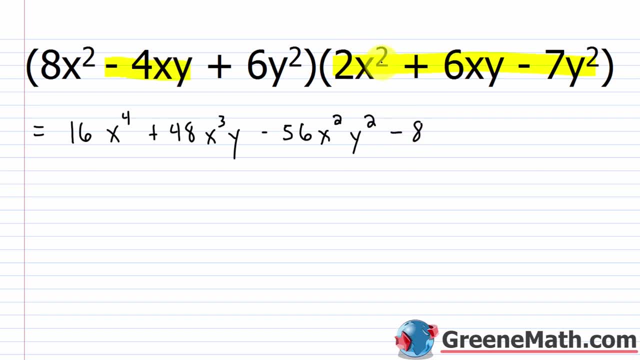 negative 4 times 2 is negative 8.. X times x squared is x cubed, and then y would come along for the ride. Then negative 4xy times 6xy, we'd have negative 4 times 6, which would be negative 24.. 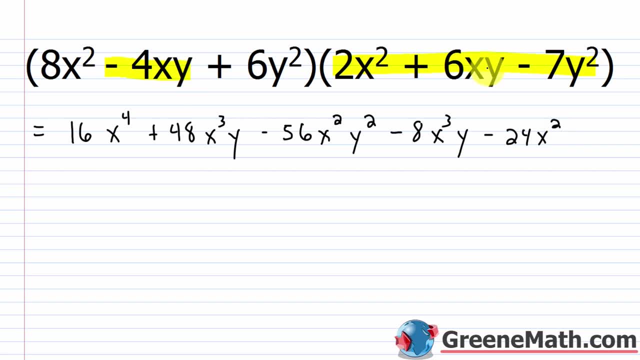 X times x is x squared. Y times y would be y squared. And let me make this two a little better Then. the last one I'm going to do here is negative: 4xy times negative, 7y squared. Negative: 4 times negative: 7 is positive 28.. 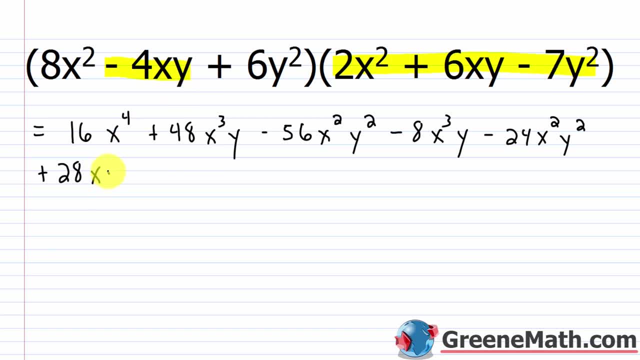 X would come along for the ride, and then y times y squared would be y cubed. All right, let's erase this. Now we're on the final term of the first polynomial. So 6y squared times 2x squared. 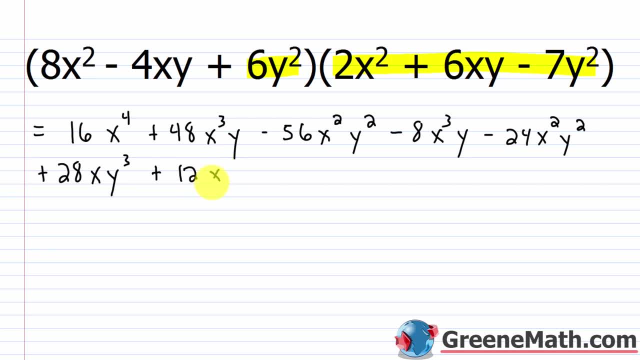 6 times 2 is 12. So plus 12. And then you'd have x squared, y squared. Then we have 6y squared times 6xy. 6 times 6 is 36. And you'd have x. 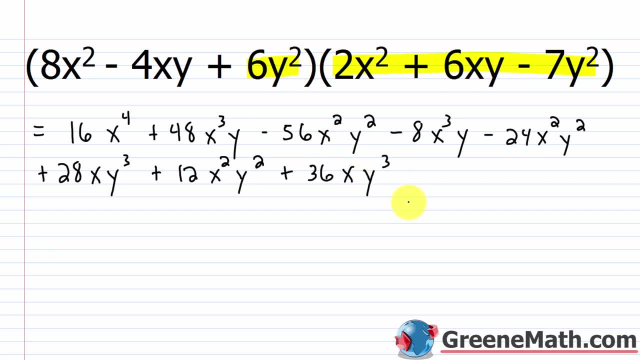 Y squared times. y would be y cubed. All right then. lastly, we have 6y squared times negative. 7y squared. We know that's negative. 6 times 7 is 42.. Y squared times. y squared is y to the fourth power. 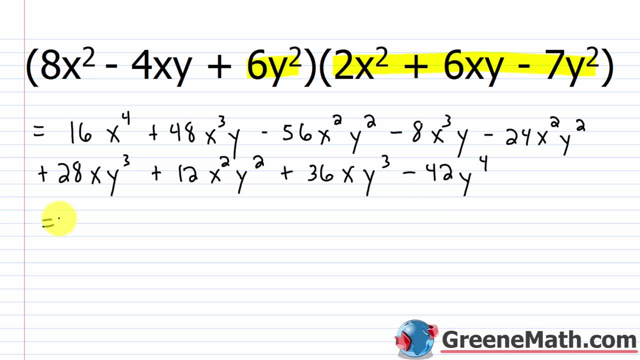 All right. So again we see how tedious this is, And even if you get into something with four terms, five terms, six terms, it just gets worse. So now I'm looking for like terms And I'm just going to start out with looking at x. 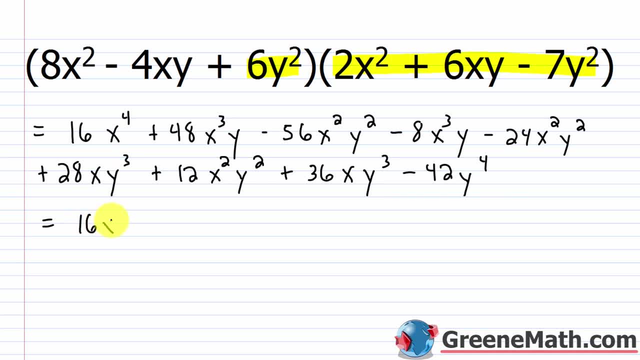 So I have 16x to the fourth power, So let's write that first. Then I have x cubed here, So do I find x cubed anywhere else? Yeah, I've got x cubed And let me erase this. 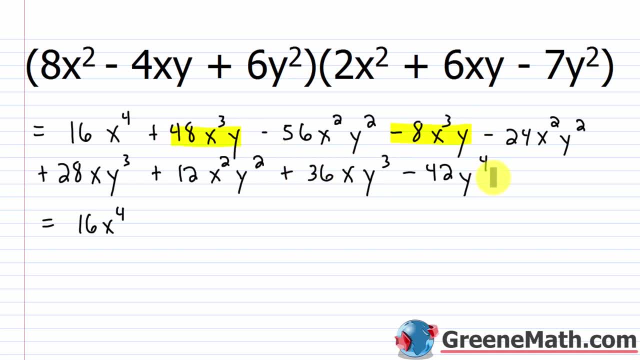 I've got the same thing here and here, So I have x cubed here. Do I have that anywhere else? No, I do not. So let's go with that. 48 minus 8 is 40. So let's put plus 40.. 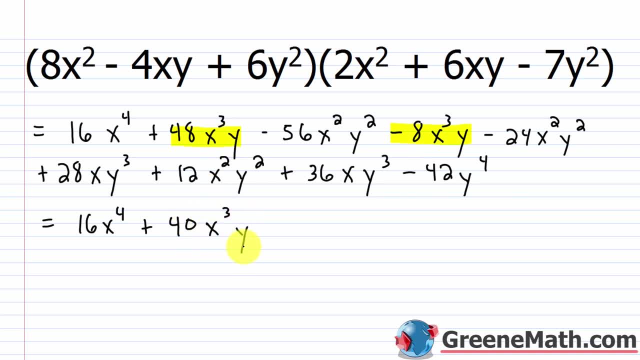 I have x cubed and then y, So let's look at x again and see what we have. So we've got x squared, y squared, x squared, y squared, So let's go with these. And then we've got x squared, y squared here. 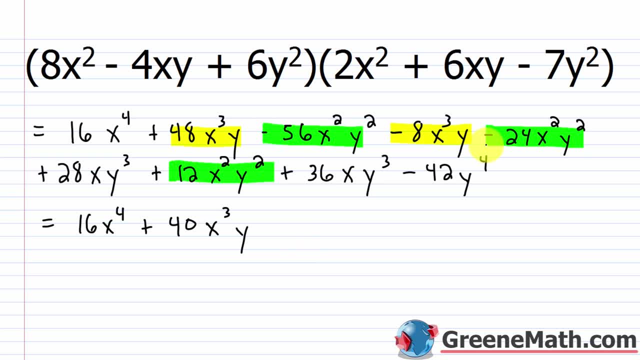 And that's all that. it appears So negative 56 minus 24 plus 12.. Well, that's going to give me negative 68.. And then, of course, times x squared, y squared, And then again, in terms of x, I've. 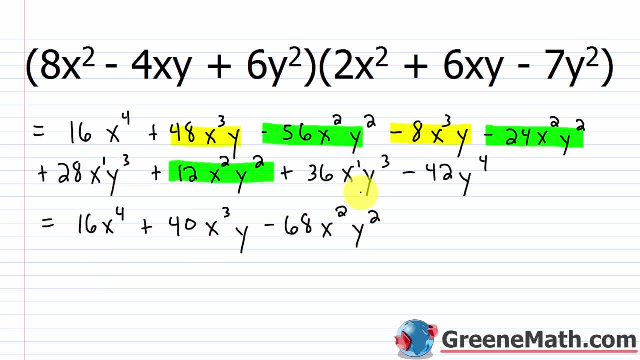 got x to the first power y cubed, x to the first power y cubed. again, Let's highlight these. And we want to combine those. So 28 plus 36 would be 64. So I put plus 64. That's x to the first power y cubed. 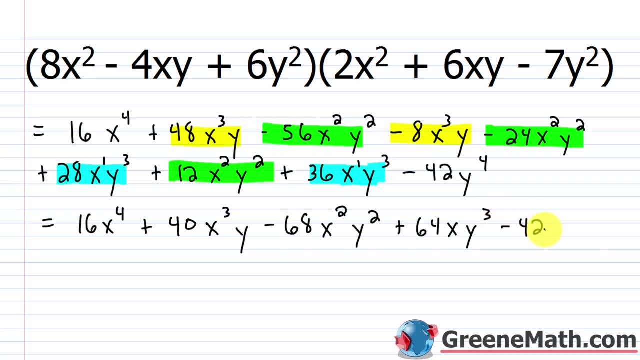 And then, lastly, I have this Minus 42y to the fourth power. Nothing to combine with that. So I've got 16x to the fourth power plus 40x cubed y minus 68x squared y, squared plus 64xy cubed, minus 42y. 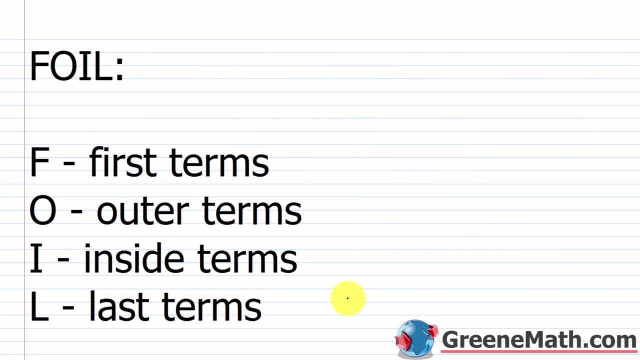 to the fourth power. All right, so now let's talk a little bit about FOIL. Now, for any of you who took an Algebra 1 course, you're very familiar with FOIL. You know that this is a method to multiply. 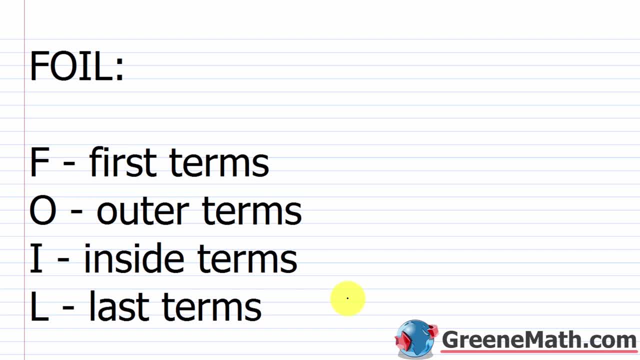 two binomials together. We can't use FOIL in any other situation, So it's only the product of two binomials. Now, FOIL just makes it very easy to keep track of what's been done, because you go in an order. 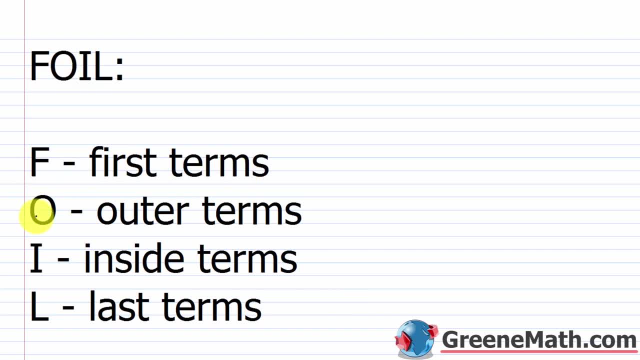 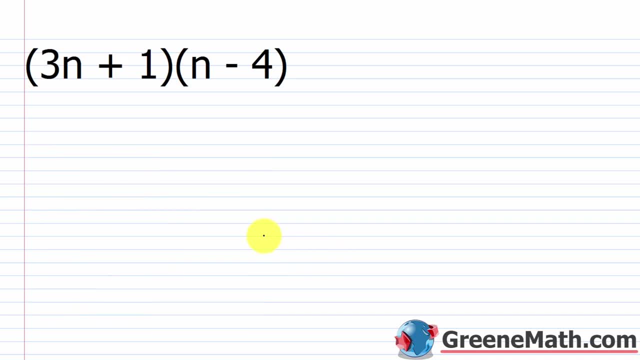 So FOIL is an acronym that stands for first terms, outer terms, inner terms or inside terms and then last terms. So as an example, here we have two binomials being multiplied together. Again, I've got two terms here. 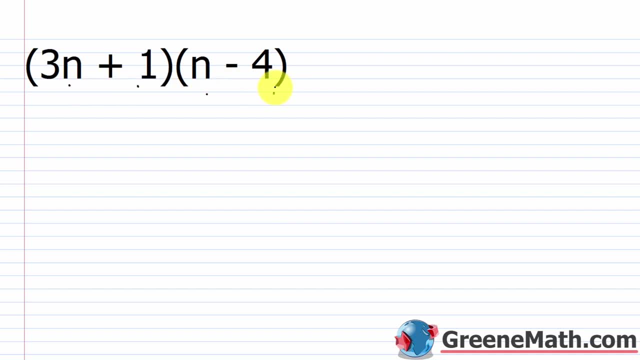 I've got two terms here. If you had a two-term polynomial multiplied by a three-term polynomial, you can't use FOIL. Or if you had a monomial times a trinomial, you can't use FOIL. It's got to be two binomials. 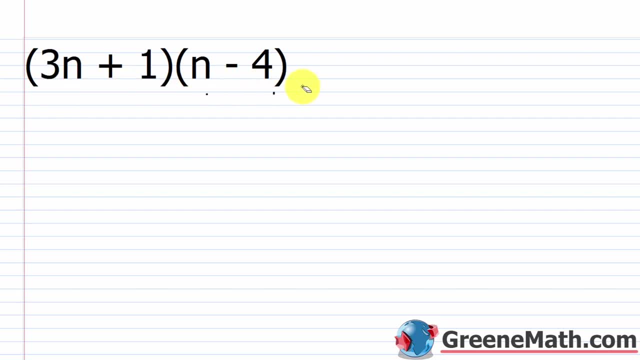 Make sure you understand that. Now, with this I'm going to use FOIL, So let's just write this out as FOIL. We'll just take it slow. So the first terms: It means the first term that appears in each binomial. 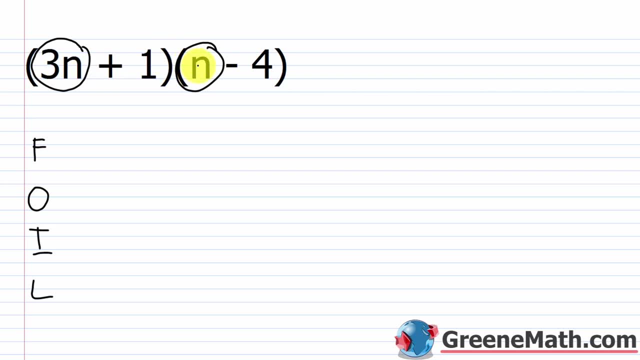 So this one times this one, So 3n times n, is 3n squared. Then you go to your outer terms. So what's outside? Well, this is outside here. This is outside here. So 3n times negative 4 would be negative 12n. 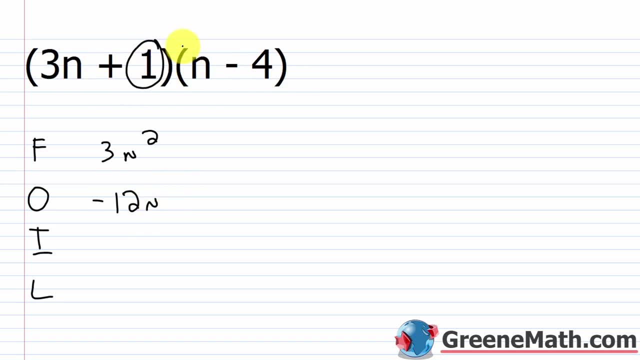 Then the inside terms. So what's inside? So you have 1 times n or just n, Then your last term. So this is last and this is last. 1 times negative 4 is negative 4.. Now you would just sum these: 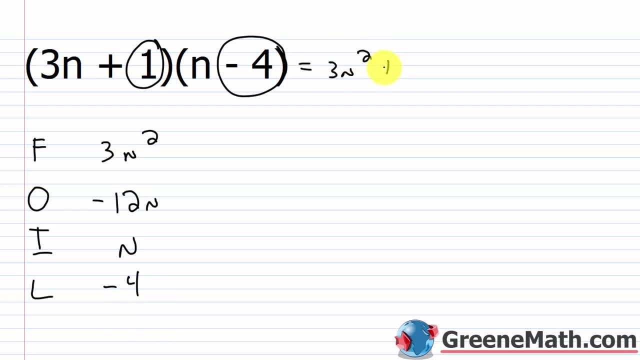 So, in other words, I would get 3n squared plus. you have negative 12n, so negative 12n plus n, and then plus negative 4 minus 4.. Now let me erase this, And if I sum these, all I'm going to do is combine the like terms that we have. 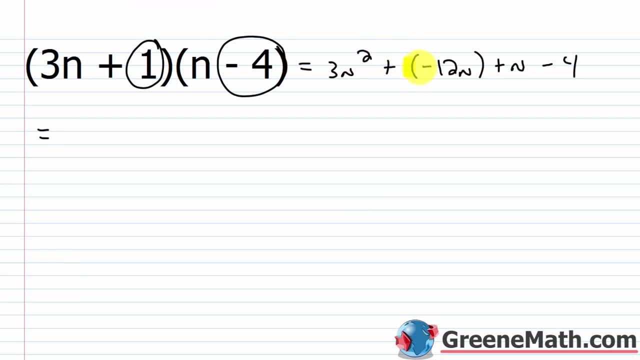 So I'm going to do this. I'm going to do this. Here's the terms that we have in our middle here. So these middle two terms can be combined. So I'd have 3n squared Negative 12n plus n is negative 11n. 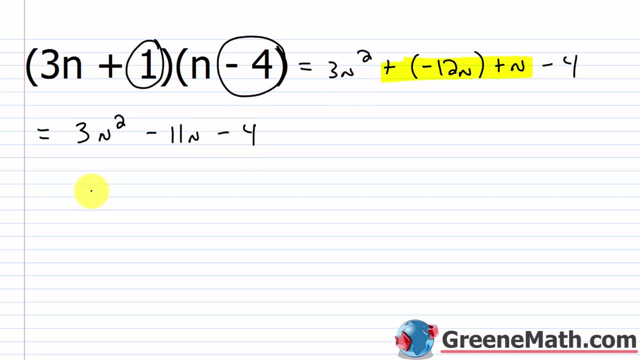 And then minus 4.. And it's just that simple. And a lot of times people can get really good at this and do FOIL in their head And they could just simply observe this and write the answer down, especially for something that's pretty simple. 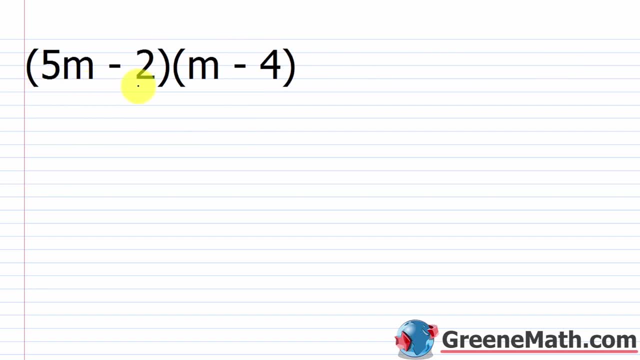 All right, let's take a look at another one. So we have 5m minus 2, that quantity times m minus 4.. So again, if I want to use FOIL, I would do my first terms. So 5m times m, that's 5m squared. 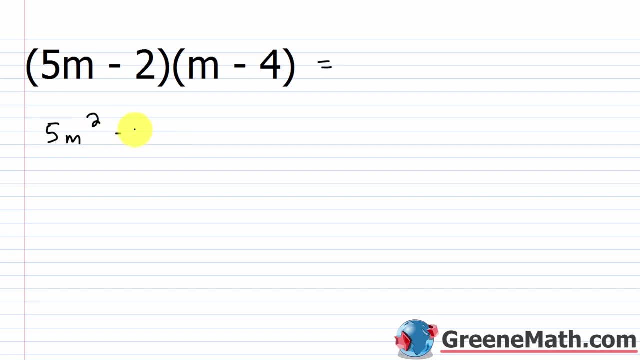 Then my outside terms: 5m times negative 4 is negative 20m. Then my inner terms: negative 2 times m is negative 2m. Then my last terms: negative 2 times negative 4 is positive 8.. 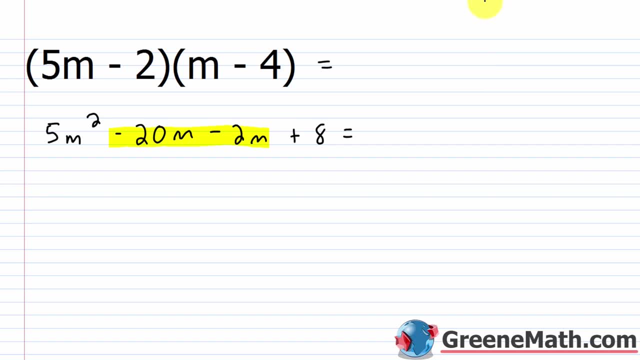 I would again combine the like terms in the middle. So I'd start with 5m squared In the middle: negative 20m. minus 2m would be negative 22m And then plus 8.. All right, as another example, let's say we have the quantity 2x minus 5y. 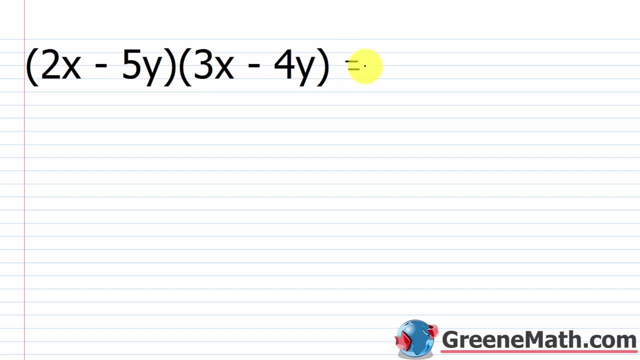 times the quantity 3x minus 4y. So again I'm going to use FOIL. So my first terms 2x times 3x would be 6x squared. My outer 2x times negative 4y would be negative 8xy. 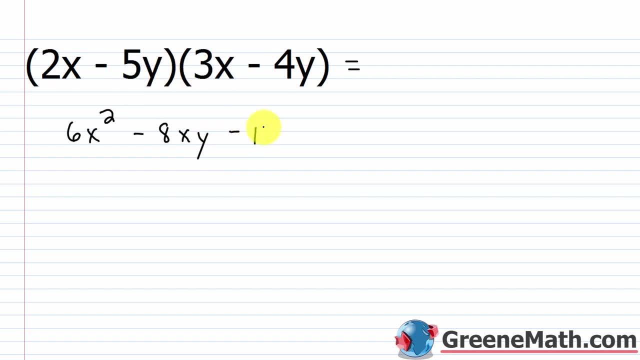 My inner negative 5y times 3x would be negative 15xy. And then my left Last negative 5y times negative 4y would be positive 20y squared. So again I'm going to combine the like terms in the middle here. 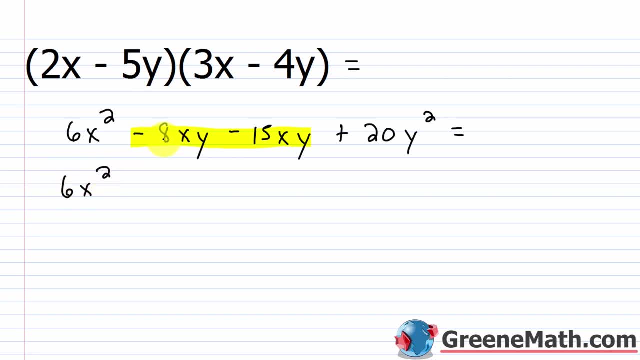 And so I'd have 6x squared. Negative 8 minus 15 is going to give me negative 23. So you'd have negative 23xy and then plus 20y squared. All right, let's take a look at one more of these. 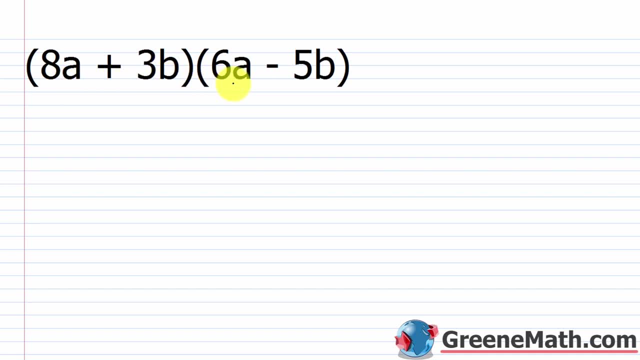 So we have the quantity 8a plus 3b times the quantity 6a minus 5b. Again, to use FOIL to start with the first terms, 8a times 6a is 48a squared. Then the outer 8a times negative 5b would be negative 40ab. 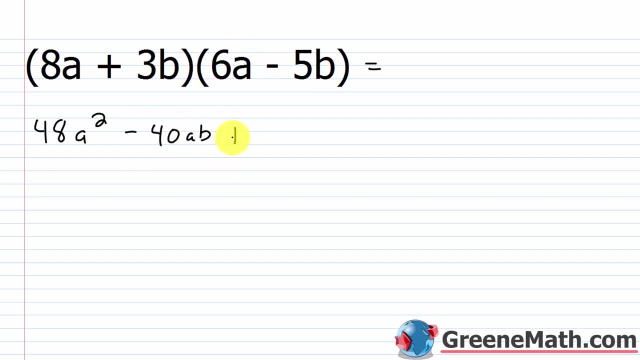 Then the inner 3b times 6a would be positive 18ab. Then the last 3b times negative 5b would be negative 15b squared. So what I want to do is I want to combine like terms in the middle. 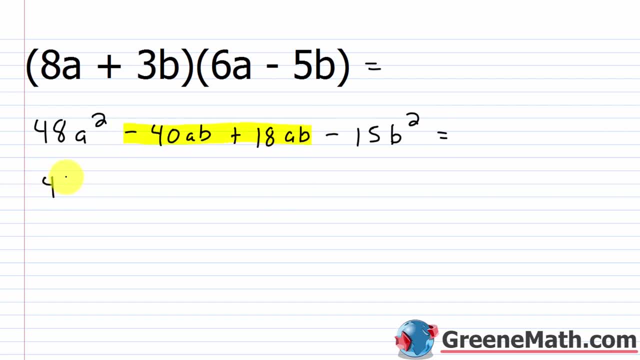 So in the middle, right there, So I'd have 48a squared. negative 40ab plus 18ab would end up giving me negative 22ab and then minus 15b squared. So I'd have 48a squared minus 22ab, minus 15b squared. 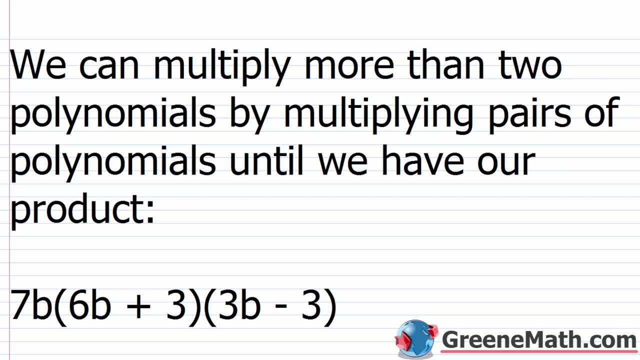 All right. so the last thing I want to talk about is what to do when you have more than two polynomials that are being multiplied. So what I have here: we can multiply more than two polynomials by multiplying pairs of polynomials until we have our product. 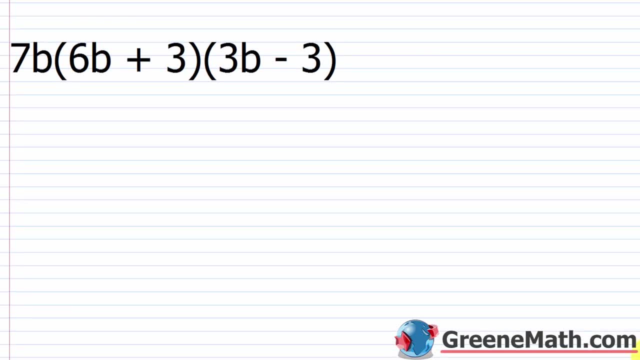 So this is the same thing as if I had, let's say, 3 times 7 times 2.. I can multiply any two together to start, and then multiply that result by the third. I could say: 3 times 7 is 21,, 21 times 2 is 42.. 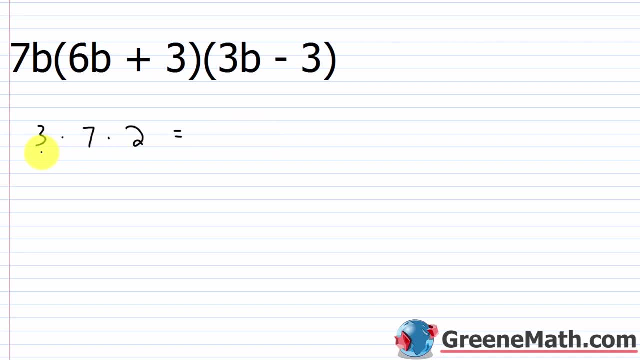 Or I could say: 7 times 2 is 14.. 14 times 3 is 42.. Or I could say: 3 times 2 is 6.. 6 times 7 is 42.. No matter how you do this, you end up with 42.. 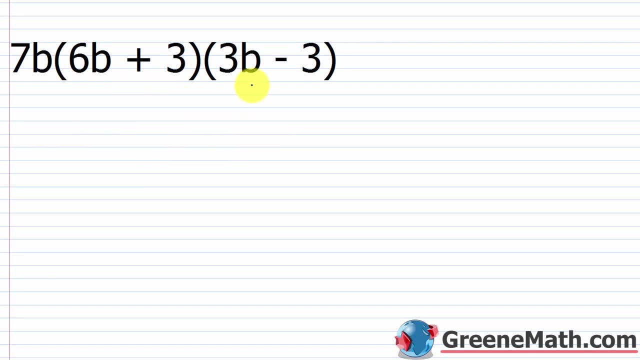 It's the same thing when we're talking about multiplying three polynomials together. I could take 7b and multiply it by the quantity 6b plus 3.. Then take that result and multiply it by the quantity 3b minus 3.. 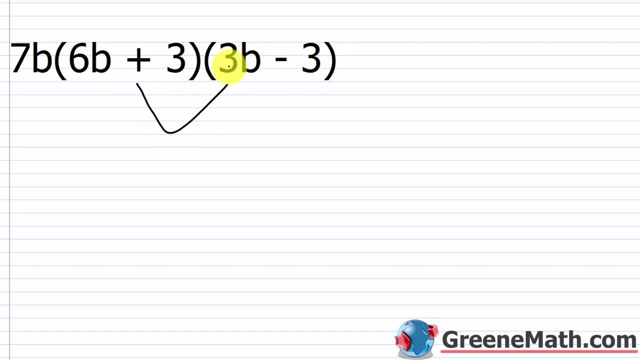 Or I could do something different. I could multiply these two together first, multiply that by 7b. Again, it doesn't matter. It does not matter as long as everything gets multiplied together. So what I'm going to do is I'm going to start out just going straight across. 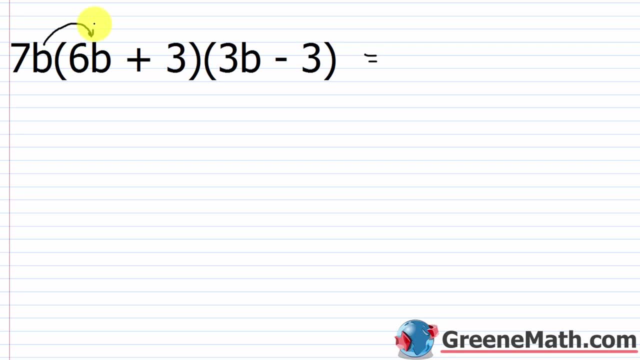 I'm going to use my distributive property and say 7b times 6b is going to give me 42b squared. Then 7b times 3 would be plus 21b. So you'd have this now: this quantity multiplied by this quantity: 3b minus 3.. 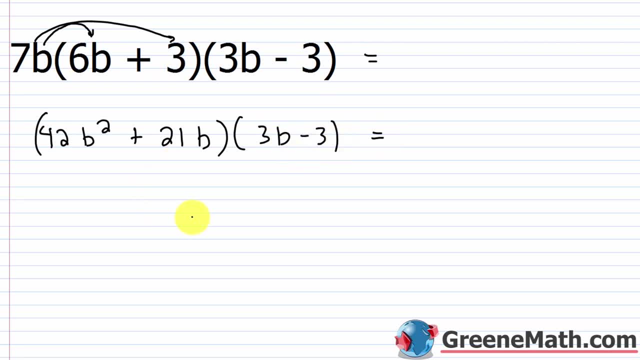 Now I've got two binomials here So I can use FOIL. So to begin, my first term is 42b squared times 3b would be 126, and then b cubed My outer: 42b squared times negative 3.. 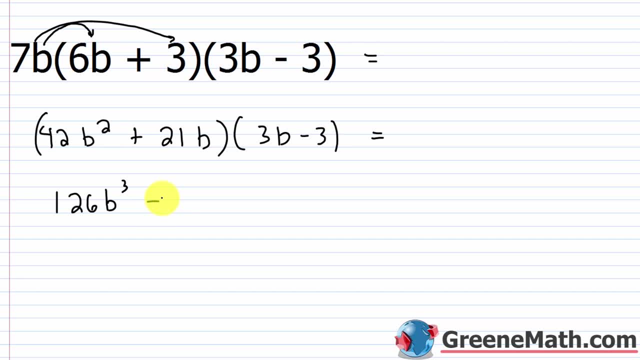 We know that's negative. Again, 42 times 3 is 126, so negative 126.. And now we just have b squared For the inside terms, we have 21b times 3b. 21 times 3 is 63, so plus 63.. 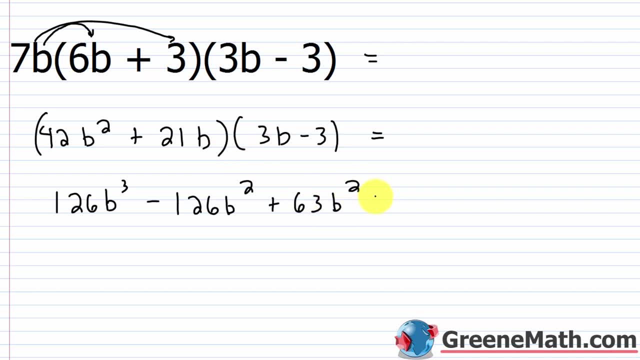 b times b is b squared. And then for the last terms, 21b times negative 3, you'd have negative 63b. So in the middle here we can combine like terms. We have negative 126b squared, We have positive 63b squared. 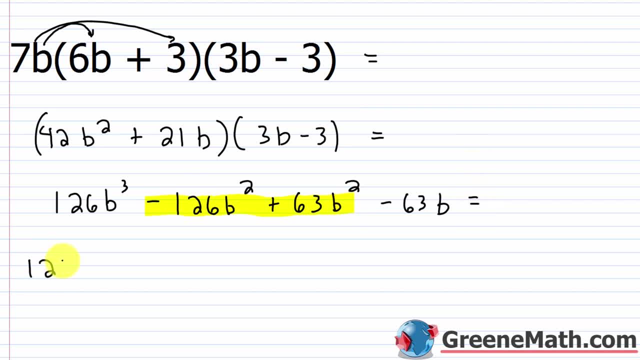 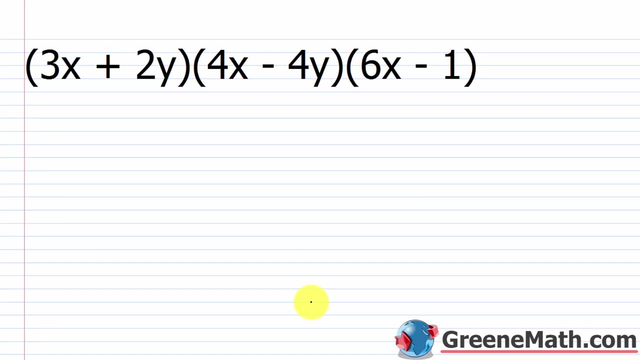 So what we have is 126b cubed, Negative. 126 plus 63 is negative 63, and then b squared and then minus 63b. Alright, let's take a look at one final problem. So we're going to multiply three binomials together. 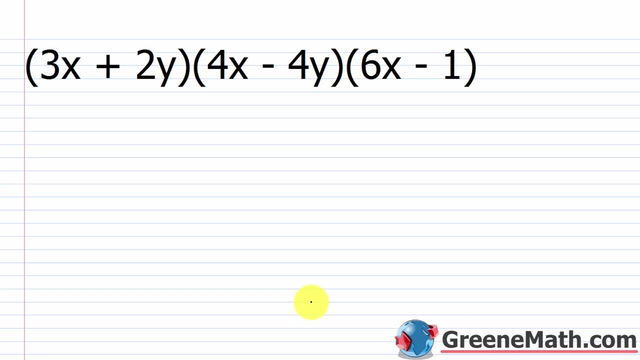 So, again, not a hard process, just something that's tedious. You're going to find the product of two of them first, doesn't matter which two, and then multiply that result by the third. So let's go ahead and start out by just saying that I'm going 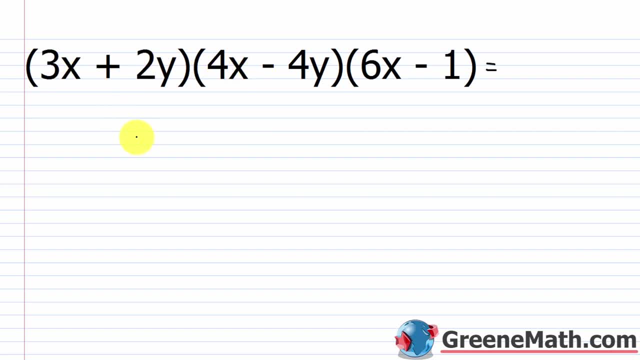 to multiply the first one by the second one. So my first terms: 3x times 4x would be 12x squared. The outer 3x times negative 4y would be negative 12xy. the inner 2y times 4x would be positive 8xy. and then for the 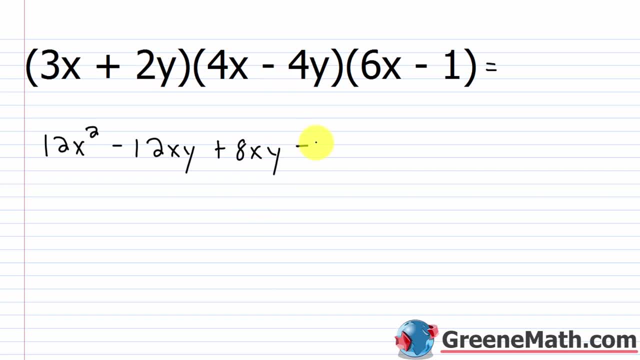 last 2y times. negative 4y, that would be negative 8y squared. Now I can combine like terms in the middle: negative 12xy plus 8xy would be negative 4xy. So this would be multiplied by this final binomial here, which is 6x minus 1.. 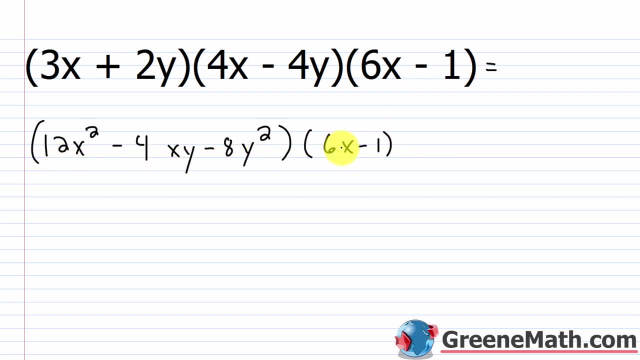 Now I can no longer use FOIL because I have a trinomial times a binomial, so I can't go, okay, first outer, inner. it doesn't work that way. So what I'm going to do is I'm going to take each term from this binomial and multiply. 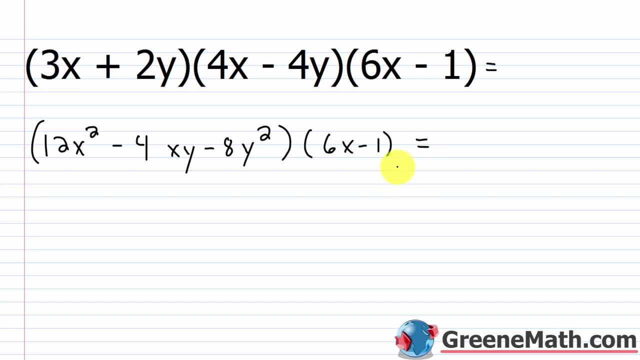 it by each term of the trinomial. So in other words, I'm going to take 6x to start and multiply it by this trinomial here. So 6x times 12xy, 6 times 12 is 72,. x times x, squared is x cubed. 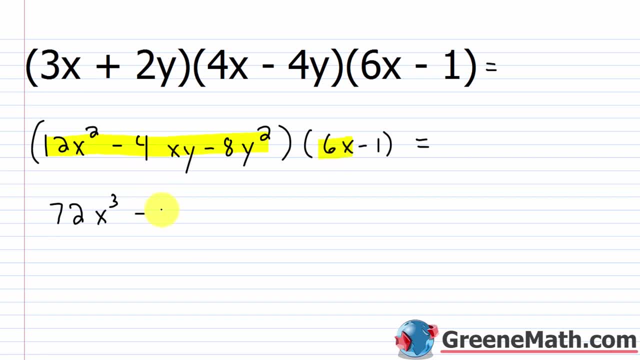 Then next: 6x times negative: 4xy, that's negative 24x squared. y, 6x times negative, 8y squared, that's negative 48xy squared. Now the next one's pretty easy. I've got a negative 1, that's multiplying this trinomial here. but multiply everything by. 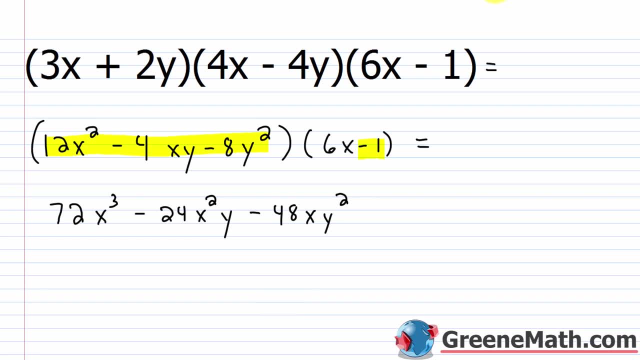 negative 1. I'm just changing the sum, So I would go through here and just say: okay, well, 12x squared will become negative, 12x squared Negative. 4xy would become positive 4xy and then negative. 8y squared would be positive. 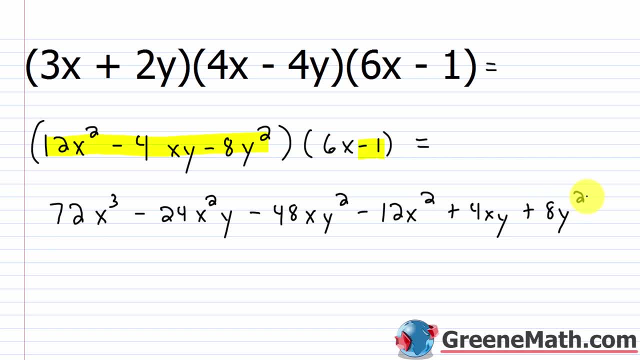 8y squared. So that's all it does. Multiply by negative 1, you're just changing the sum. So now I would just look to see if I can simplify this any further, and I actually can't. There are no like terms here. 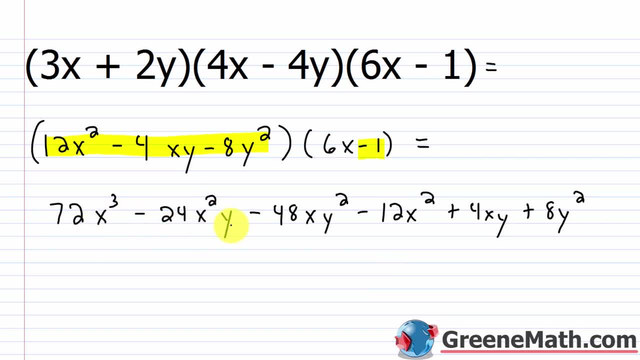 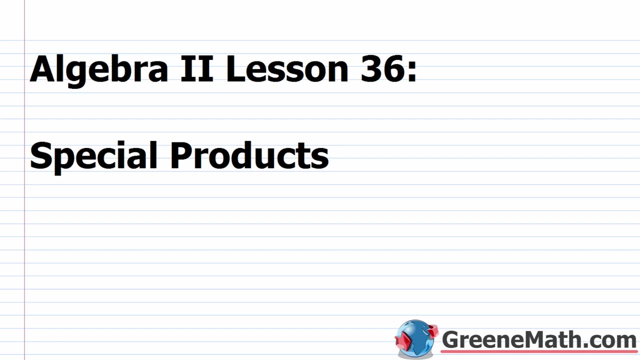 We end up with 72x cubed minus 24x squared y Minus 48xy squared, minus 12x squared plus 4xy plus 8y squared. Hello and welcome to Algebra 2, Lesson 36.. In this video, we're going to learn about special products. 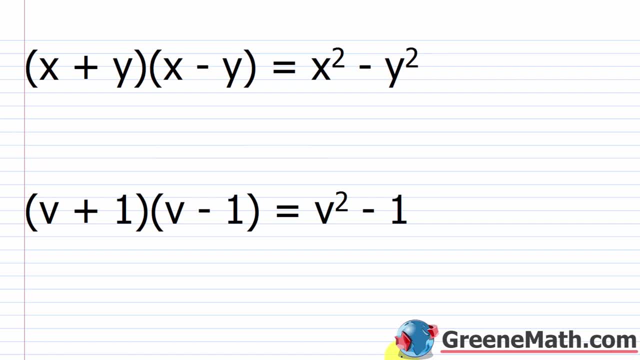 So again we've come to another scenario where, if you've taken Algebra 1, this lesson is nothing more than a refresher for you. but it's an important refresher because we're going to look at polynomial products that occur so frequently that it's extremely useful. 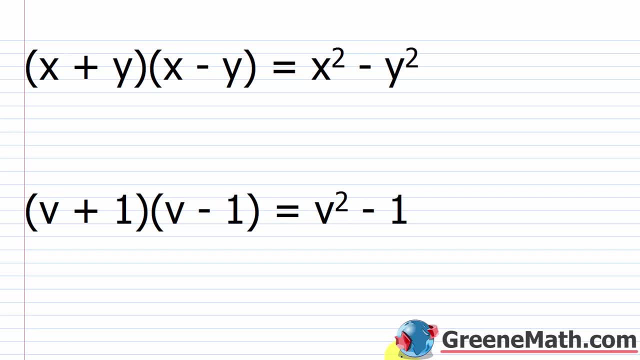 to memorize the pattern associated with these products, And you might do it just to be faster on your homework or on your tests. but I can tell you when you start taking these standardized tests like the SAT, the ACT, or even if you're 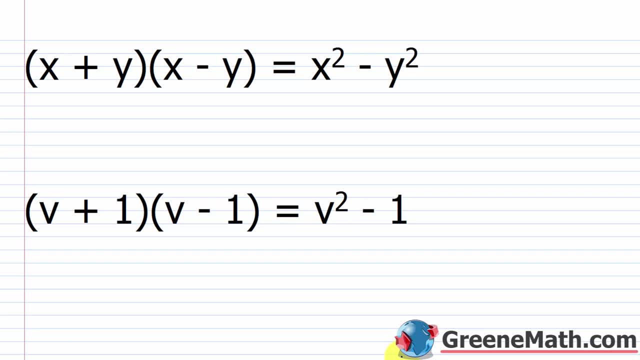 going to grad school, even if you've graduated from college already. you want to take your GRE or your GMAT, or whatever you're taking. those tests are designed with a time limit that, in some cases, requires you to be able to spit out these products very, very quickly. 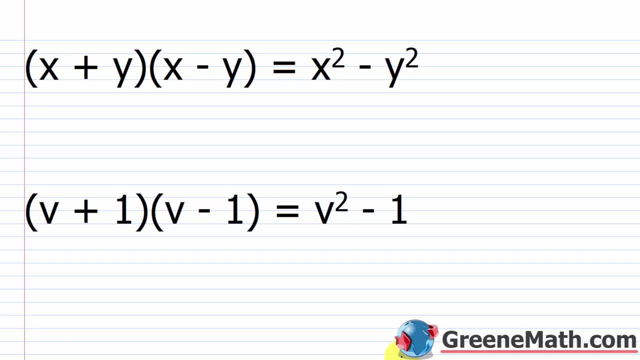 Okay, So this is just something you can use to do that. So I want to start out with something that's very, very basic, something that most of you know. So if I have something like the quantity x plus y times the quantity x minus y, we can. 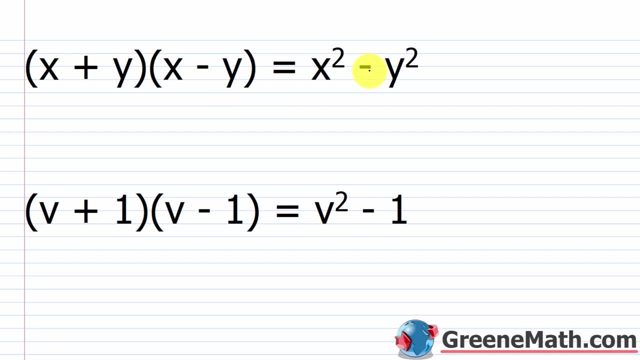 say: this is equal to x squared minus y squared. Now, first I want to do this with FOIL and then I want to show you why it ends up this way and how we can translate something generic like this to our actual problem. So if I did FOIL here, 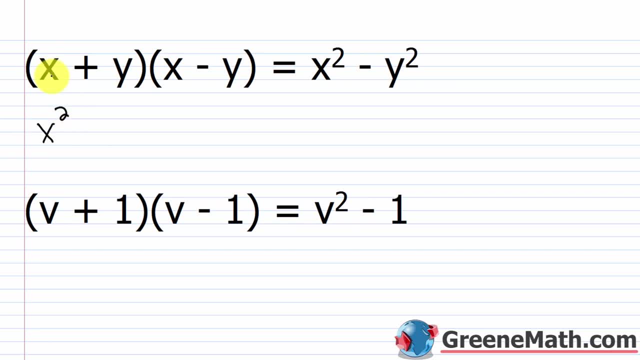 If I did x squared minus y squared, So if I did FOIL here, If I did x squared minus y squared, So if I did x times x, that would be x squared. and if I did x times negative y, that would. 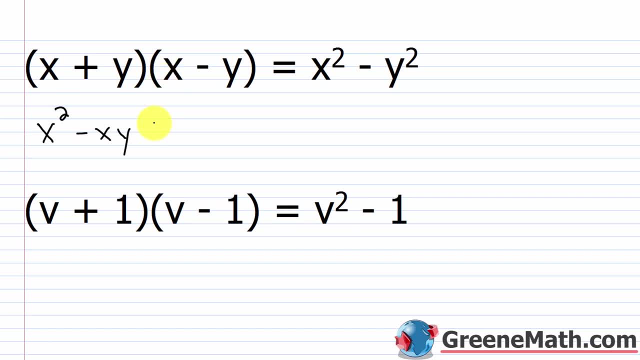 be minus xy, and if I did y times x, that would be plus xy, and then if I did y times negative y, I'd have minus y squared. So what happens with this? the middle two terms are going to cancel and I'm left with 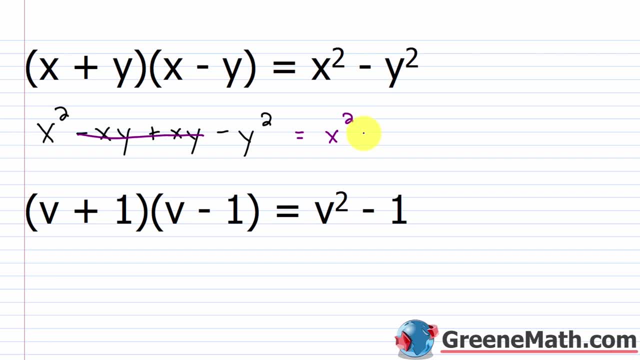 x squared minus y squared. So this is x squared minus y squared. So you're looking to make sure that you have the same term in the first position of each binomial. So I have an x and an x. I've got to have different signs, I have a plus and a minus, and then I've got to have 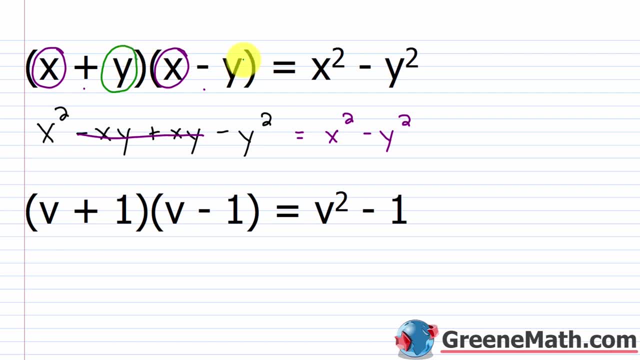 the same term in the second or last position of each binomial as well. I have a y and a y, So if it fits that pattern, you can go ahead and say that you have the first guy or the first item that's going to be squared, then we're subtracting away the second or the last. 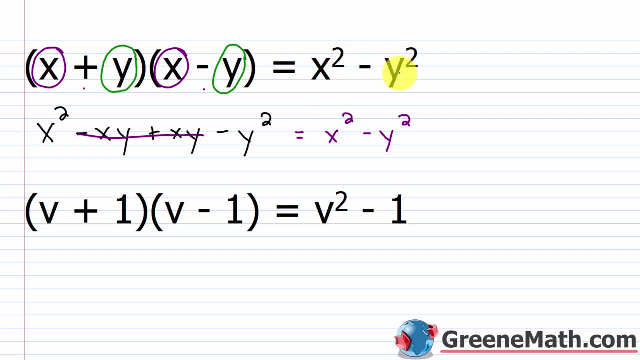 guy squared, And this is referred to as the difference of two squares. I have something like this: I have something squared here minus something squared here. So as another example, let's say you saw the quantity v plus 1 times the quantity v minus. 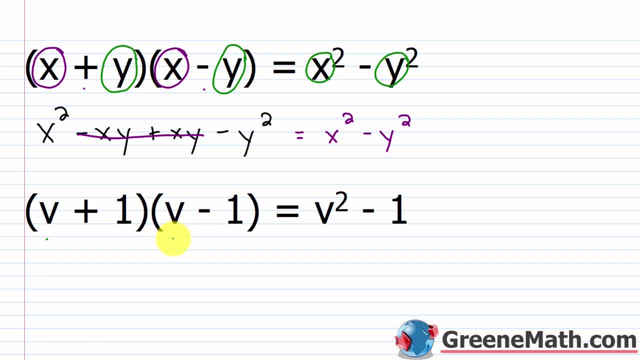 1.. Well, again I think about, this is v, this is v. So same item in the first position of each, then this is 1, this is 1.. Same thing in the second position or last position of each. then I have a positive and. 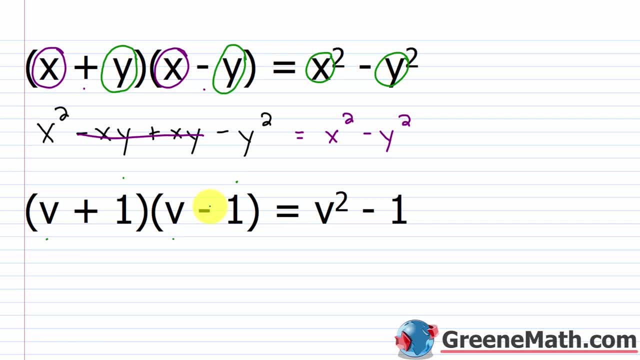 a negative. so I have different signs. So, without going through and doing FOIL, I can say: I have the first guy which is v squared. that's what I have there. Subtract away the second guy which is 1 squared. 1 squared is 1, so I get v squared. 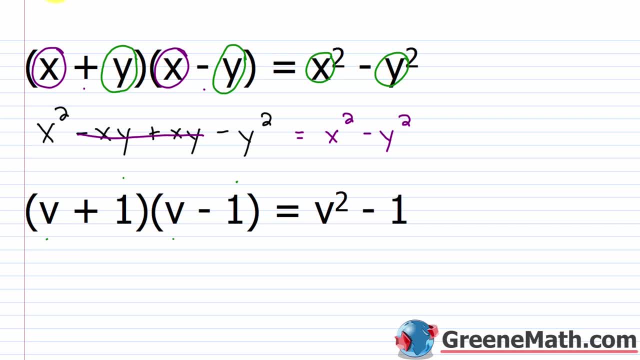 minus 1.. And again, if you want to prove this to yourself, you can use FOIL: v times v is v squared, The outer would be minus v, The inner would be plus v. so we know those would cancel And the last would be negative 1, right 1 times negative 1 is negative 1.. 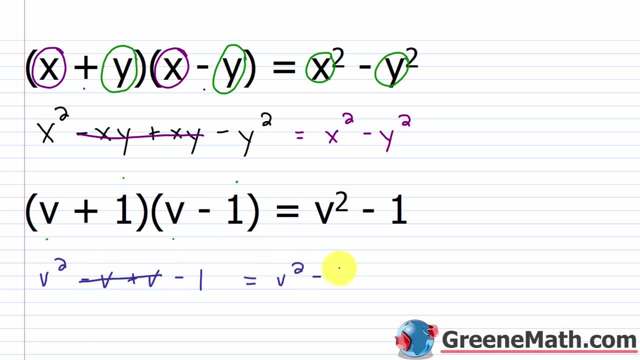 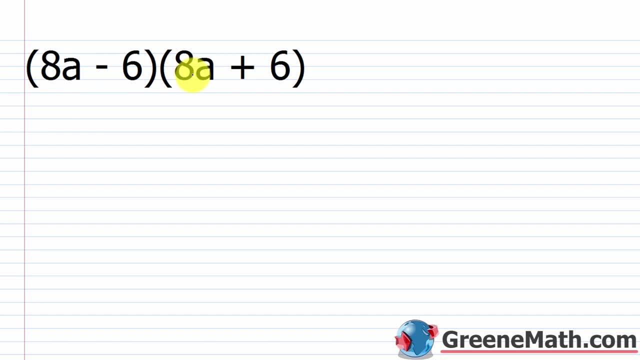 So again, these cancel. I end up with v squared minus 1.. All right, Let's look at some more examples. All right, So let's say we had something like the quantity 8a minus 6 times the quantity 8a plus 6.. 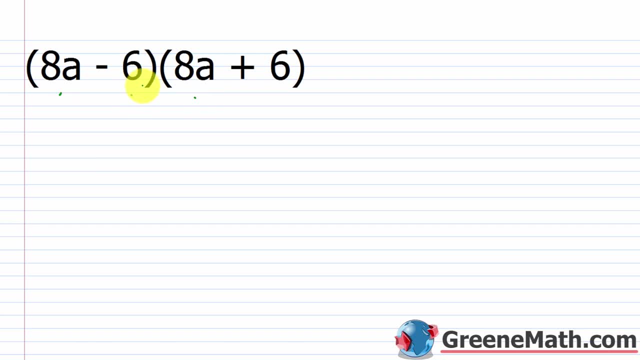 So it's the same thing here. I have 8a and 8a, then I have 6 and 6, and your signs are different. I have minus and I have plus, So I don't have to go through and use FOIL. 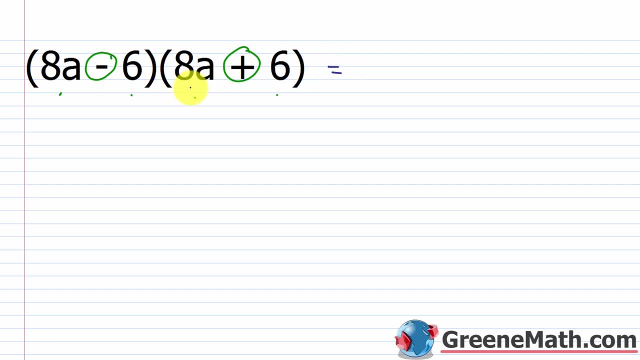 I can do this very, very quickly by just squaring 8a, So 8a squared. okay, you've got to be careful that you're squaring this whole thing, this whole term here. You can't just do 8a squared like that. 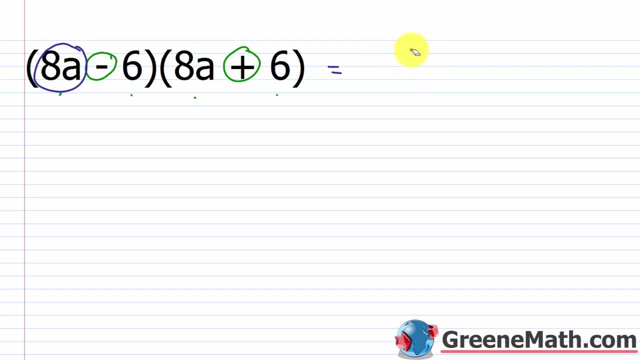 I see that all the time. That's not going to work. I've got to square that whole term. So I would square 8.. 8 squared is 64.. I would square a. That's just a squared. Then minus. I'm going to look at my 6 and that's going to be squared. 6 squared is 36.. 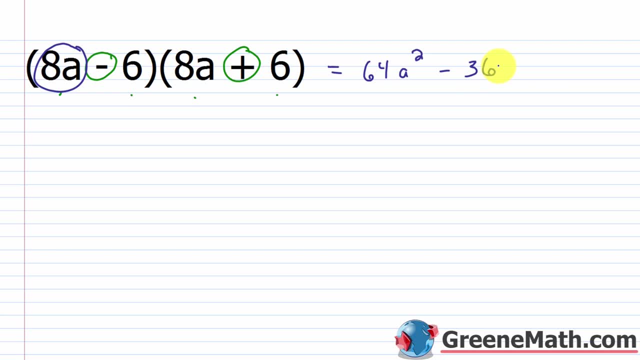 So just that quickly, without doing FOIL or anything else, I know my answer is 64a squared minus 36.. And again we can prove it to ourselves: 8a times 8a is 64a squared. The outer 8a times 6 would be positive 48a. 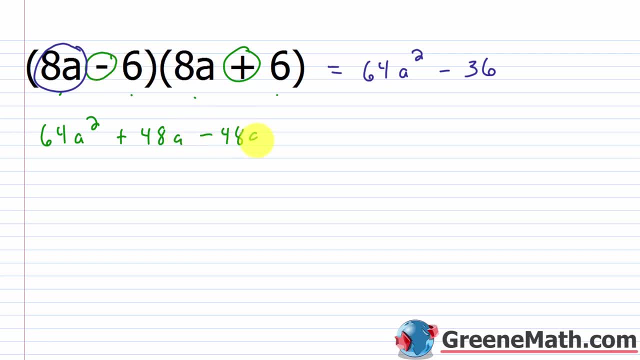 The inner negative 6 times 8a would be minus 48a, And then your last negative 6 times 6 would be minus 36.. So again you can see that these middle two terms are going to cancel. Positive 48a and negative 48a would cancel. 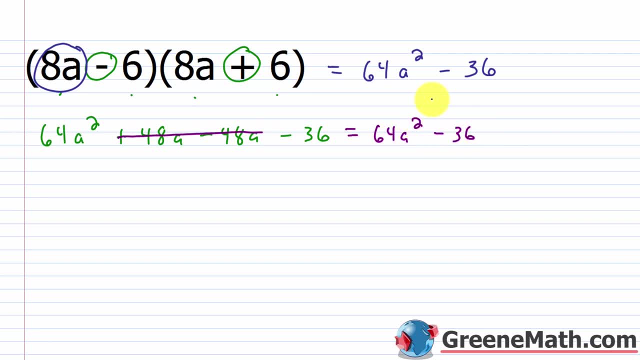 So 64a squared minus 36 is what you are left with. So just a much quicker way to do this versus using FOIL. Let's take a look at another one. So we have the quantity negative 6x minus 3y being multiplied by the quantity negative. 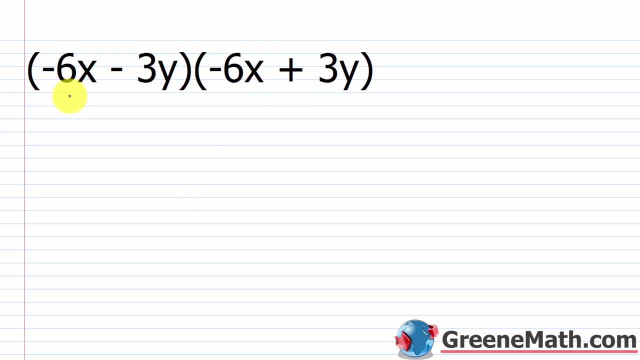 6x plus 3y. So again, I'm looking at a negative 6x here and a negative 6x here. I'm looking at a 3y here and a 3y here. Now the signs are different. 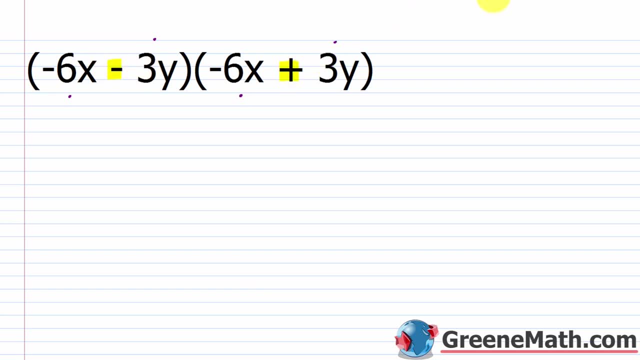 I have a negative and I have a positive. When I do my pattern, again, I'm thinking about the first thing that occurs. So this right here. Normally I'm not including the sign when I'm thinking about the second one. In this case I need to include that negative when I think about negative. 6x. 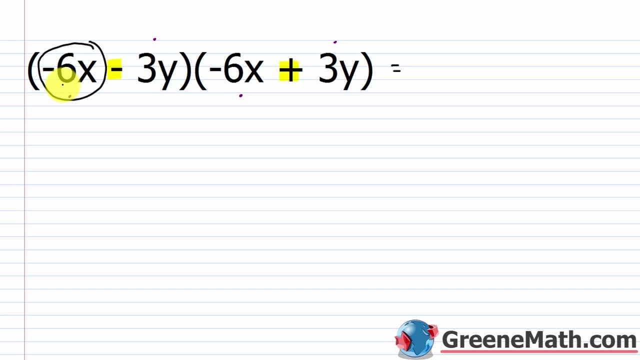 I can't just leave it off, So I would square that. So if I squared negative 6x, it would look like this: So that negative is inside the parentheses, so it's basically negative 1 squared, which is 1.. 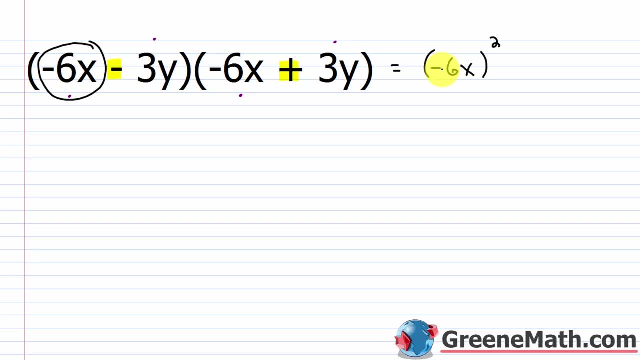 6 is squared, 6 squared is 36.. And x is squared. 6x squared is just x squared. So this is 36x squared. Then I'm subtracting away What is in the second position here, It's 3y. 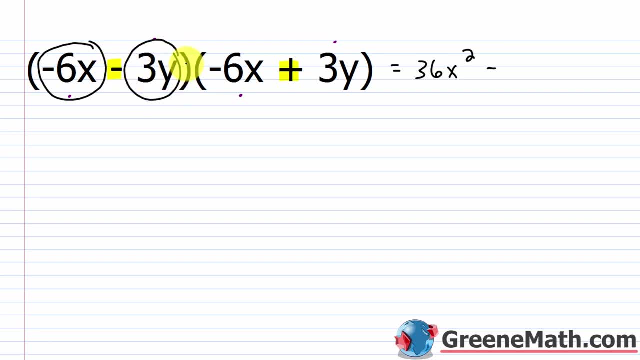 Again, when we think about what's in the second position, I never think about the sign, I just think about this right here. So 3y- If I squared 3,, I'd get 9.. If I squared y, I'd have y squared. 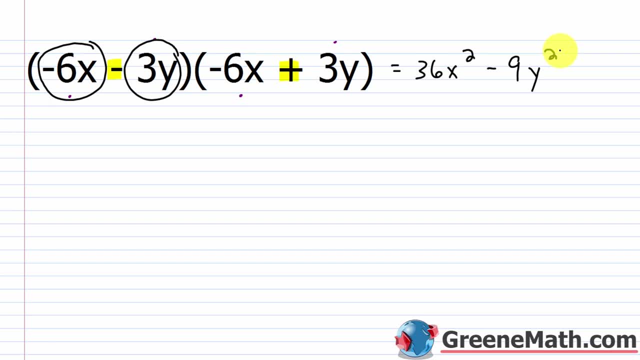 And boom, there's my answer: 36x squared minus 9y squared. Just that quick. So this one kind of the trap is to make sure that you include the sign when you think about that first term. All right, let's take a look at one more of these. 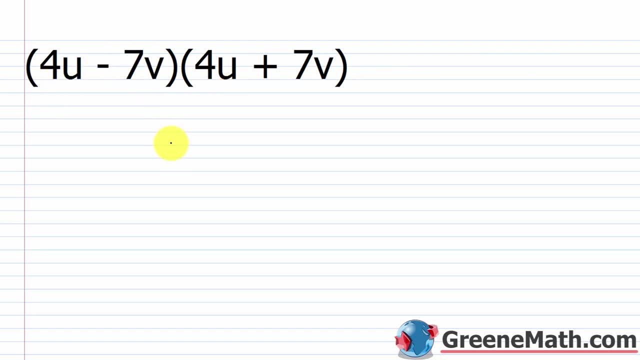 So suppose you have the quantity 4u minus 7v and you multiply it by the quantity 4u plus 7v, So I would take this guy right here, this 4u, and I would square it. So 4 squared is 16.. 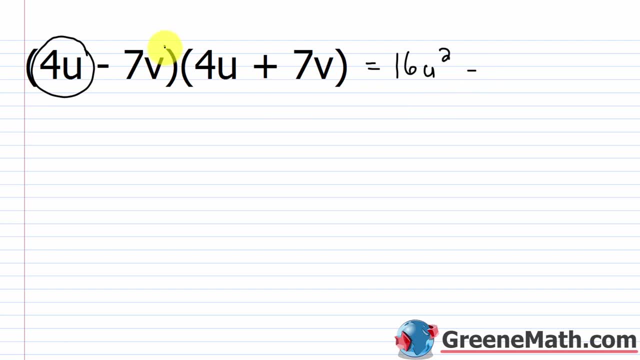 u squared is just u squared, Then minus. Take this guy right here and square it: 7 squared is 49. And v squared is 49. And v squared is just v squared. And then again, boom. just that quick I have my answer: 16u squared minus 49v squared. 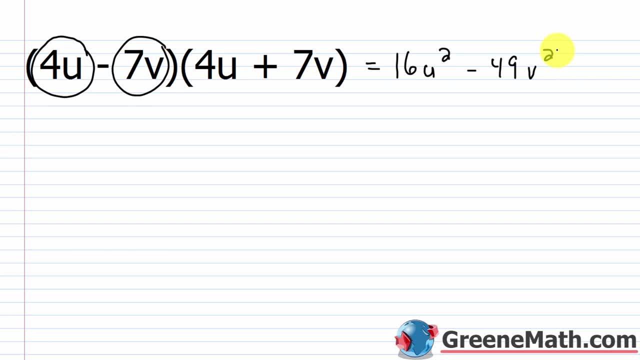 So again, we're kind of done with this section. I just want to recap and talk a little bit about this for a second. You're looking for this pattern where you have the same thing in the first position of each. In this particular case, it's 4u and 4u. 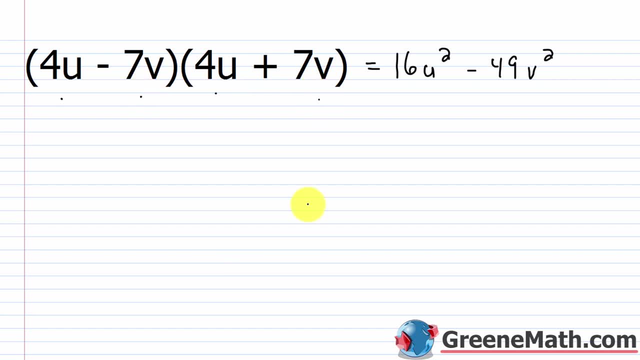 Then the second position of each has the same thing, So 7v and 7v, And then your signs are different. You have a negative and you have a positive. So that leads to this: The first guy, which is 4u squared, minus the second guy, which is 7v squared. 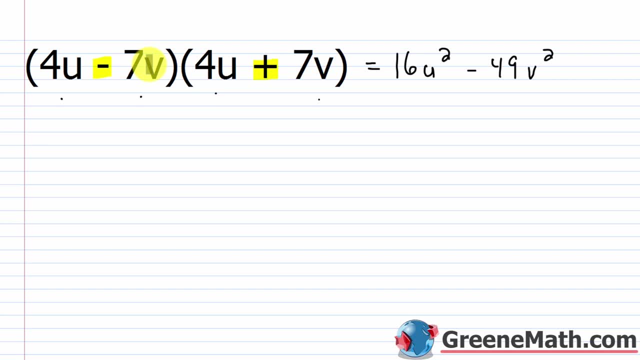 So you just memorize that pattern. You can put it on a flash card or something where you can flip through. memorize it As you do your homework, as you do your tests, as you get into your standardized exams. this is going to be very beneficial for you. 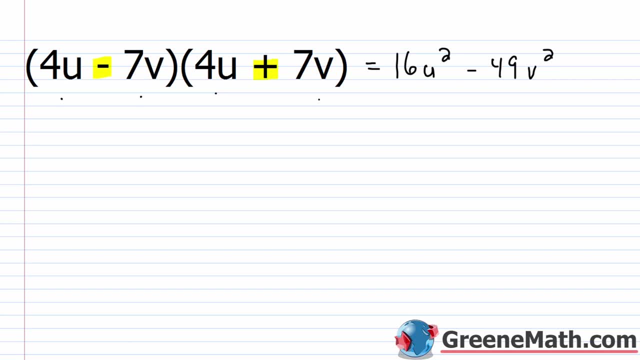 All right, Let's look at a different pattern. Let's look at a different section now. All right. So the next thing I want to talk about is the square of a binomial, And we have two different scenarios. So we have the quantity x plus y squared. 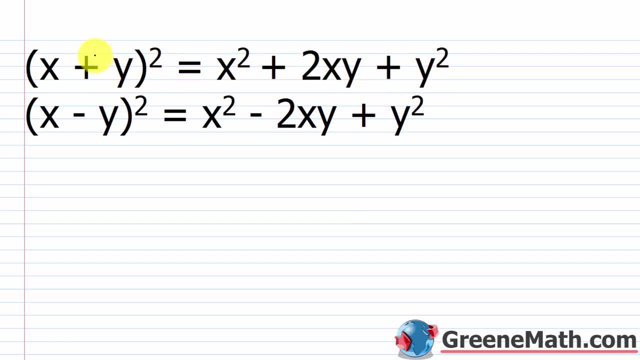 This leads to x squared plus 2xy plus y squared. So notice that when you have a plus sign here, you have a plus sign here and here. okay, So if I have this scenario, I don't need to really think about the signs. 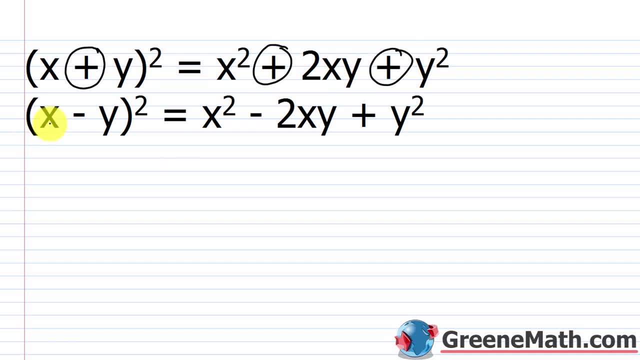 Everything's going to be a plus Now. in the other scenario we have the quantity x minus y squared. I have x squared. I have minus 2xy plus y squared. Here I have a minus in the middle, and so that leads to a minus in front of the second term. 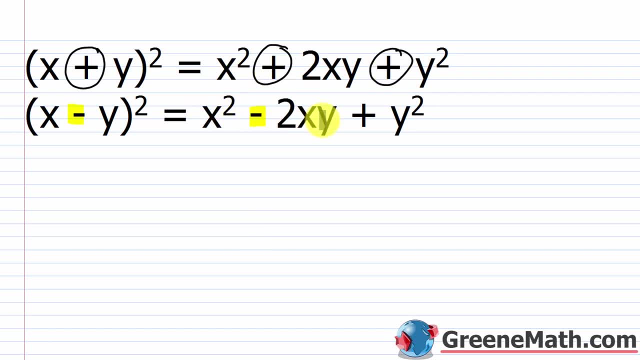 So everything else is the same. It's x squared minus 2xy plus y squared. The terms are the same. It's just this one sign that's different. okay, So it's very easy to memorize this one and it's very easy to apply it. 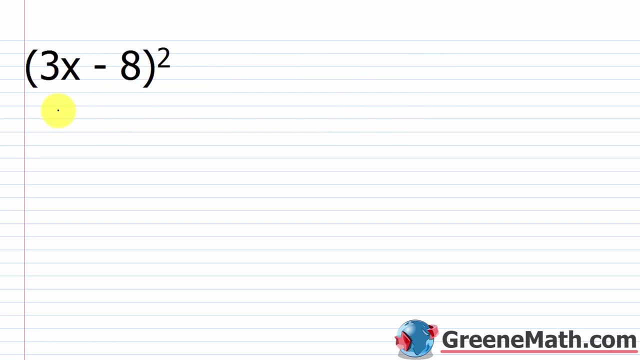 Let's take a look at an example. All right, So we start out with the quantity 3x minus 8, and this is squared. So this is a binomial squared. So what would I do here? Well, let me just write the pattern that we should know. 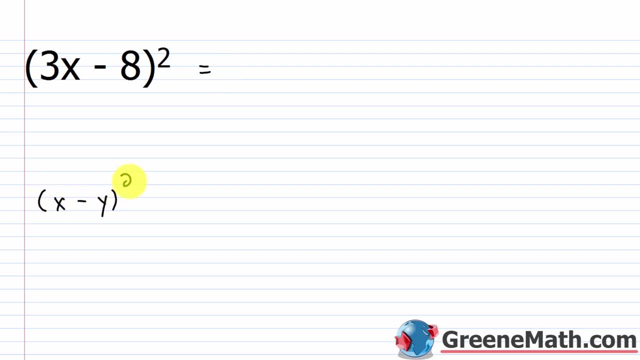 So if we do x minus y, that quantity squared, it's the first guy squared, So it's x squared. Then remember we have a minus in front of the second term because we have a minus here. Then it's 2 times x times y. 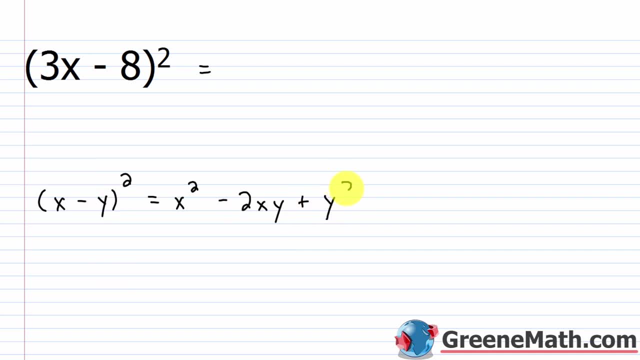 Then it's plus this guy squared, So y squared, So just match that pattern, okay. So if I take the first guy and I square, So 3x, and that's squared Again, you've got to make sure you square the 3 and the x. 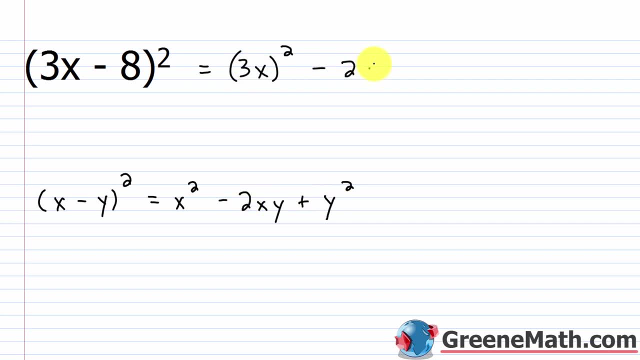 Then we would subtract away. You have 2 multiplied by x times y. So x and y just represent the first term and the second term here. So 2 multiplied by 3x multiplied by 8.. Okay, Then the next thing we have is plus y squared. 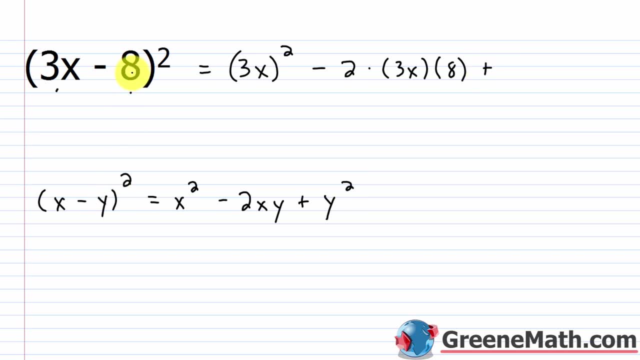 So I'm going to add to this Over here, I'm going to add to that, And then the last thing we're going to do is we're going to add to this minus y squared, which is a minus, So 8 squared. 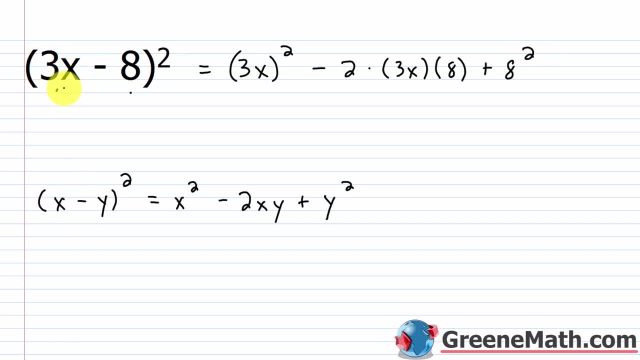 That should just be it. So it's 1 squared. Now we're going to add to that And the number's in the last position, which is 8 squared. So 8 squared, And this may take you a few times to kind of get it down. what represents what? 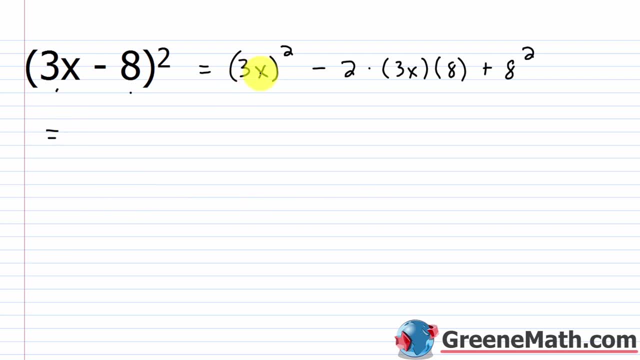 But x in this case is the first term. So that's representing 3x. here the first term Y represents the second term would be 9. then x squared is just x squared, and then we're subtracting away. we have 2 times 3. 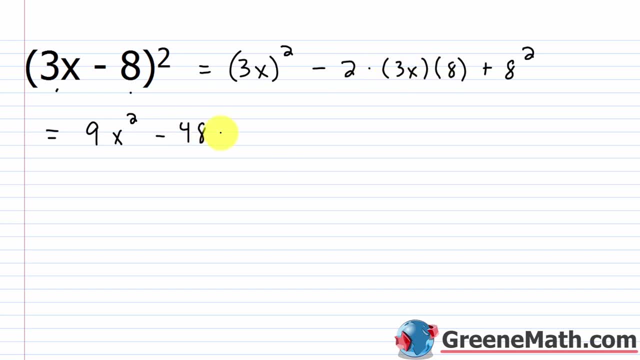 times 8, 2 times 3 is 6, 6 times 8 is 48, and then times x, and then, lastly, plus 8, squared is 64. so we get 9x squared minus 48x plus 64, and just really quickly, I'm going to prove to you that. 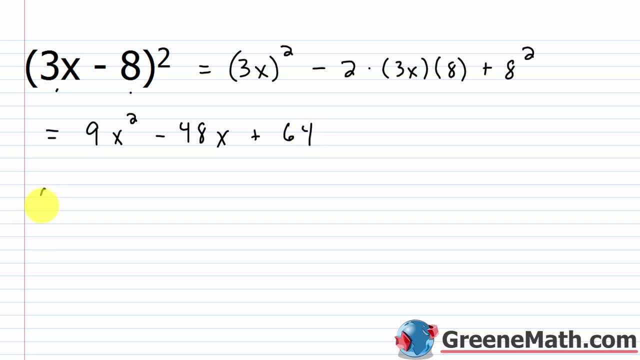 this works and I'm going to show you how much longer it takes. so if I had 3x minus 8, that quantity, if it's squared, I'm multiplying it by 3x minus 8. again, don't make the mistake of saying the quantity 3x minus 8 squared is equal to 3x squared minus 8 squared. that's wrong. 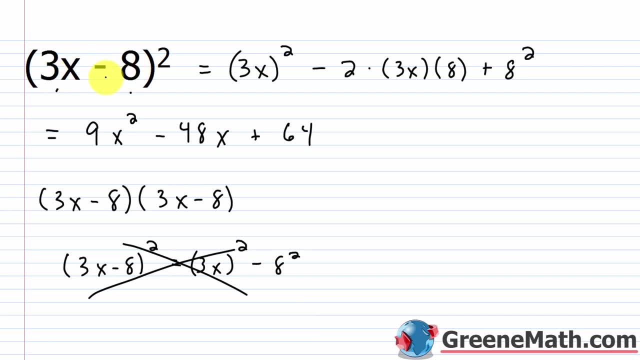 okay, please don't make that mistake. this has to be expanded out. all right. so once we have in this format, we can use: FOIL 3x times 3x is 9x squared. the outer 3x times negative 8 would be negative 24x. the inner negative 8 times 3x would be negative 24x, and then the last negative 8. 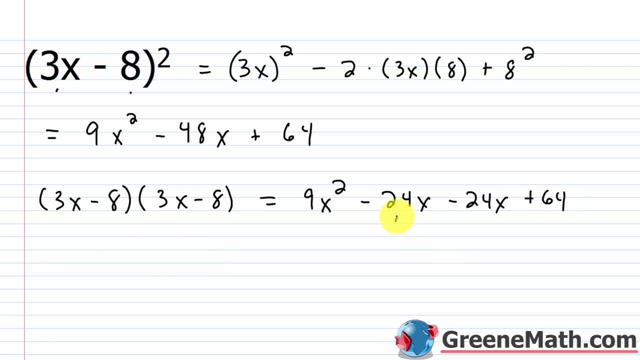 times negative: 8 is positive 64. you can see, you can combine like terms in the middle, so you would end up with 9x squared minus 48x, right, negative 24x minus 24x is negative 48x, then plus 64. 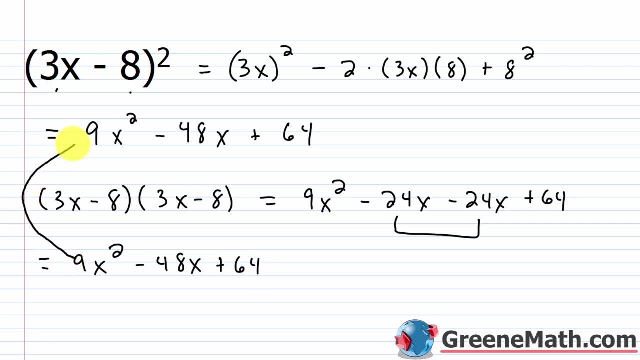 now you can see that this answer is the same as this answer. we just got this answer more quickly and we're going to do the same thing again. so we're going to do the same thing again quickly, because we used a pattern right. we recognized how we could get the answer. we applied. 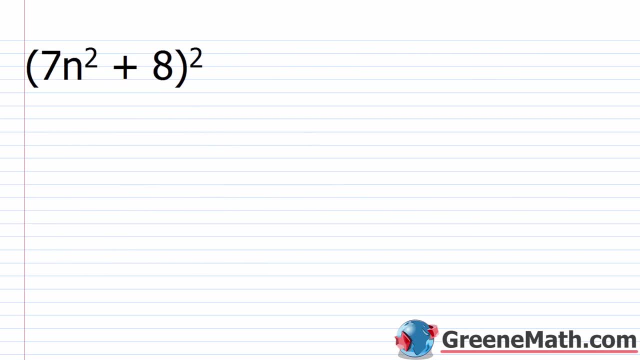 it. we got it very quickly. all right, let's take a look at another one. so we have 7n squared plus 8, that quantity, and it's squared. so again, if I think about x plus y, that quantity squared, this would be what the first guy squared, so x squared plus 2 times x, times y plus the last guy. 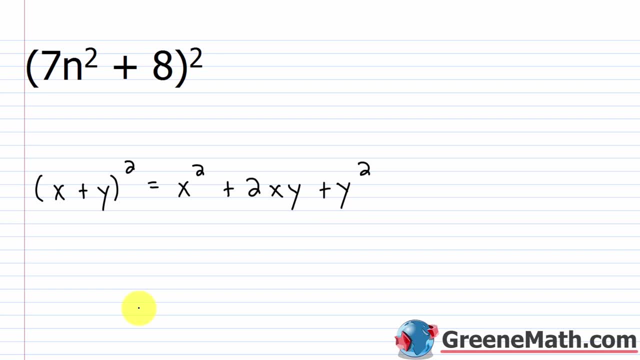 squared, and so we're going to do the same thing again, so we're going to do the same thing again, so we're going to do the same thing again. and so, the way I actually remember this, I take this guy and say, okay, this is squared, and I know this is squared, so that goes at each end. then I remember. 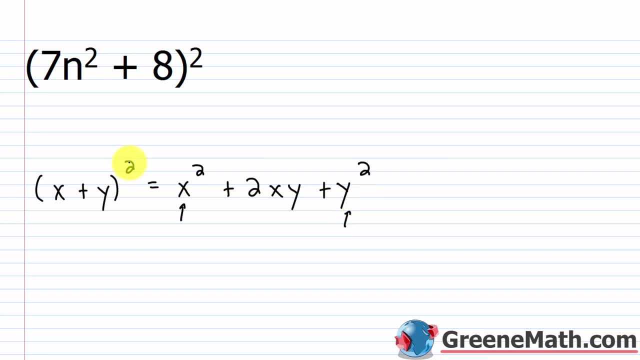 my exponent is 2. that's involved in a multiplication in the middle. so I just say, okay, well, I have 2 times x, times y. that's how I get the middle part 2xy. that's what works for me. I'm not sure what will work for you, but you can certainly try that now if I go through and try to apply this. 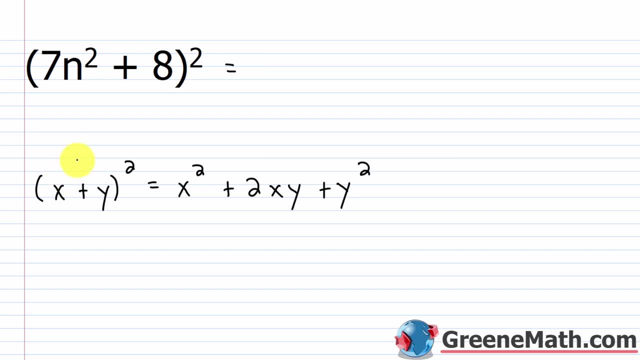 again, I have to match things up. so in this case x, which is the first term here, represents 7n squared, which is the first term here. So those match up. Then y, which is the second term here, matches up with 8,, which is the second term here. 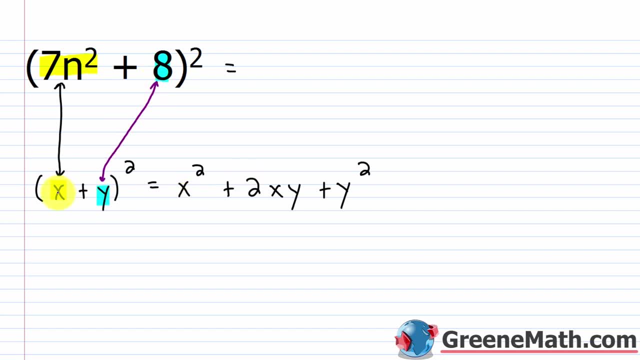 So those match up. What I'm going to do is just say, okay, in this one I have the first term squared, So 7n squared will be squared. Then plus I have 2 times the first term, times the second term. 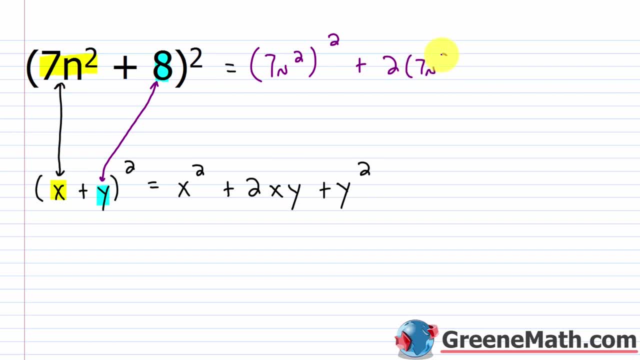 So 2 times 7n, squared, times the second term, which is 8.. Then plus y squared, So it's the last term squared, In this case, that's 8.. So 8 squared, All right, so let's erase this. 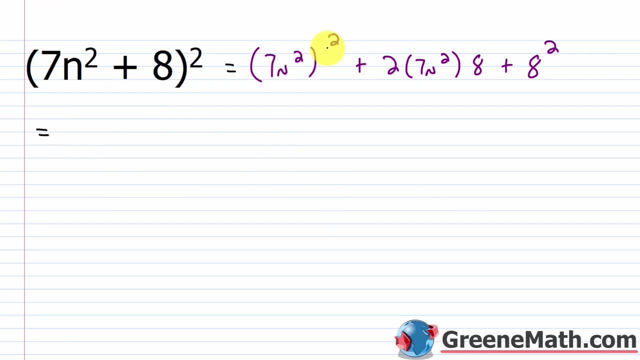 And let's just crank this out now. So if we have 7n squared squared, 7 squared is 4n squared, 49n squared squared: Power to power rule. So n stays the same. Multiply 2 times 2, that's 4.. 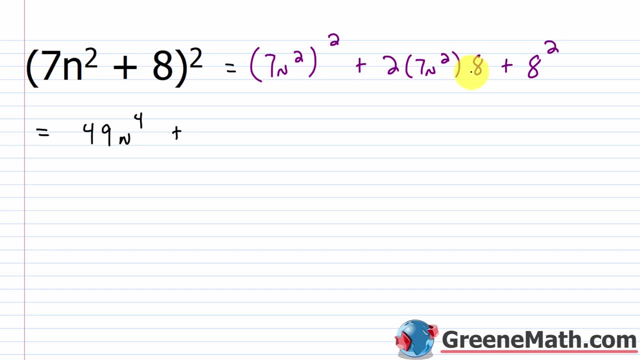 Then plus, you'd have 2 times 7 times 8. I can do 2 times 7 first. that's 14.. 14 times 8 is 112. So this would be 112.. And then times n squared. 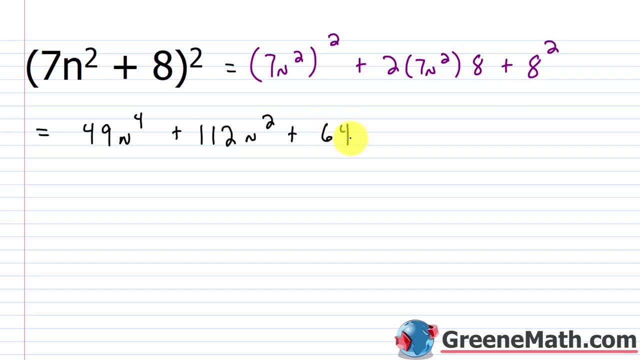 Then lastly, plus, if we have 8 squared, that's 64. So we end up with 49n to the fourth power, plus 112n squared plus 64.. All right, let's take a look at another one. 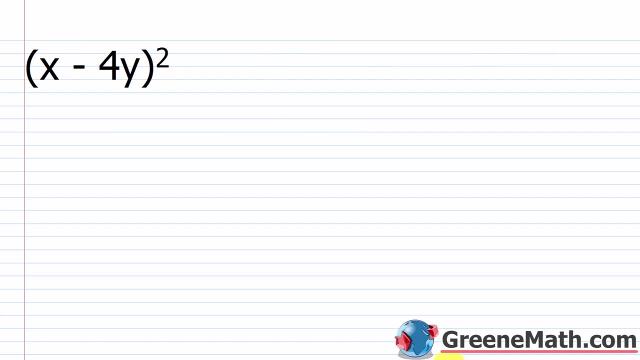 Let's suppose we had x minus 4y and this quantity is squared. So I'm going to write out my pattern and I'm going to go with x minus y, that quantity squared. So we should know at this point it's what. 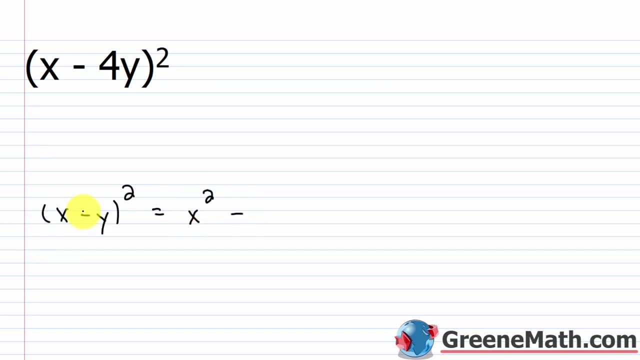 It's x, the first term squared, then minus. Remember, if you have a minus here, you have a minus in front of the second term, 2 times x times y, 2 times x times y, And then plus, the last term squared, y squared. 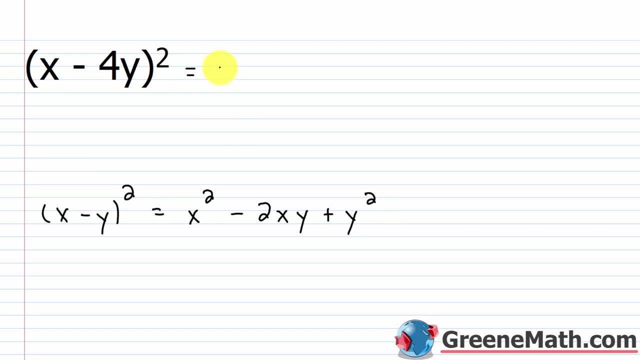 So just apply that here The first term squared, So x is squared, minus 2 times the first term times the second term, So 2 times x times 4y, and then plus the last term squared, So 4y squared. 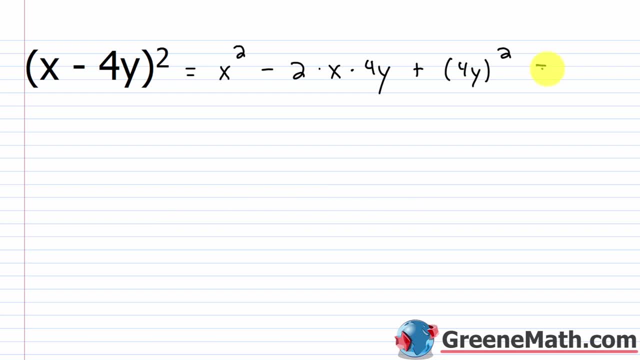 OK, we can erase this now, We don't need it. And so we'd have x squared minus 2 times 4 is 8.. So you'd have 8xy, And then plus 4 squared is 64.. And then plus 4 squared is 16, y squared is y squared. 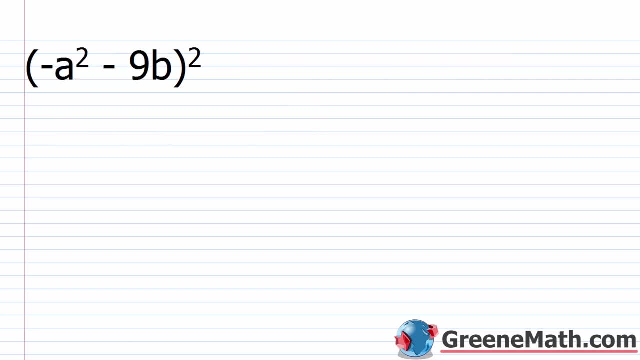 So you get x squared minus 8xy plus 16y squared. All right, let's take a look at one more of these. So I have the quantity negative a squared minus 9b, and this is squared. Now, this one's a little tricky and I'm going to get to that in a second. 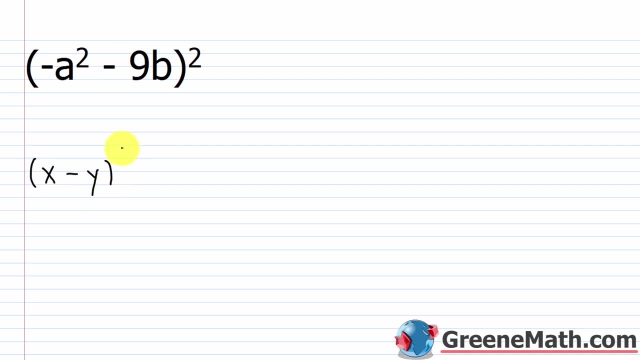 Again, if I have a subtraction in the middle, I use this formula: So x minus y, that quantity squared, This is x squared Minus 2xy Plus y squared. Now what makes this tricky is this negative right here, this negative a. 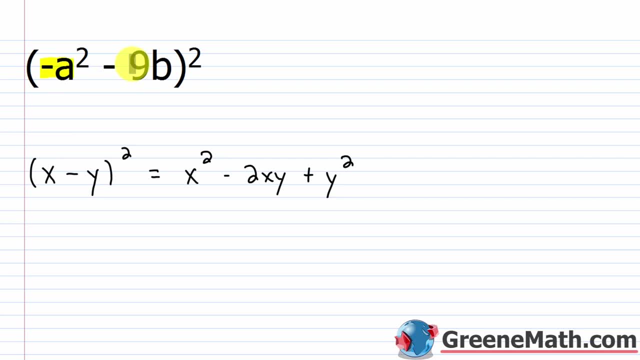 Normally we have a positive there, right? We don't think about our signs, We just use whatever's there. If you have a negative here, you've got to account for that by putting it in, OK. So that's what makes it tricky. 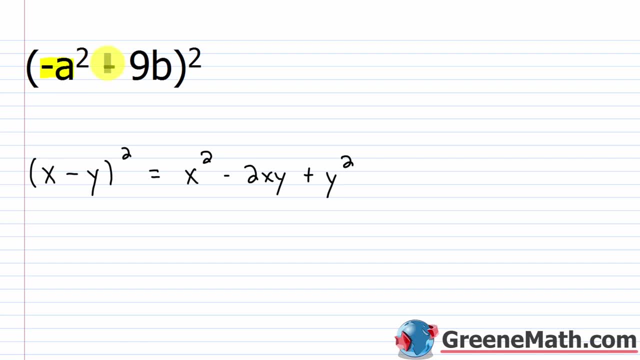 A lot of students say, OK, I'll just put an a squared in there. Or a lot of students will throw this negative in there when they think about 9b. right, This sign right here in the middle, It's already figured in for you. 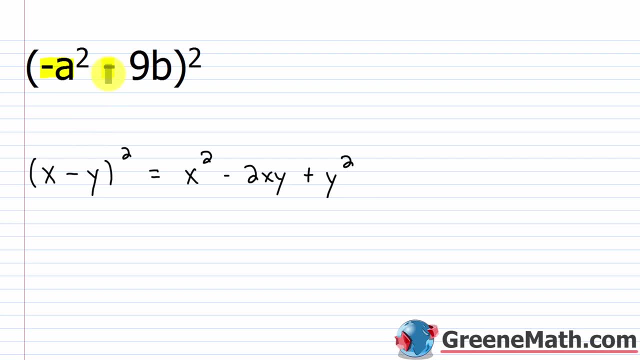 So you never need to use it. OK, You never need to think about it. If I have a negative that's thrown at me there, though, I do need to put it in, OK. So that's the difference. So what I want to do here, I want to say: I have the first guy squared. 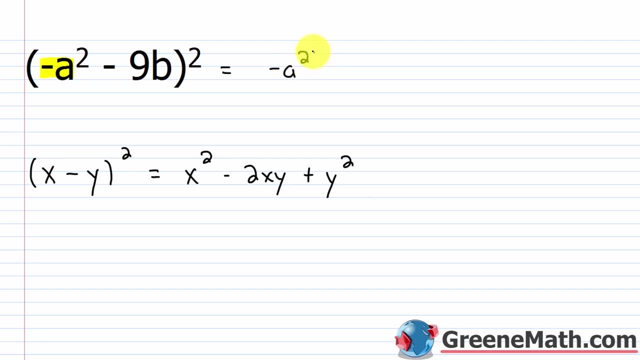 So the negative a squared the whole thing. So that's going to be squared. Then I subtract away 2 times the first guy. Again, I've got to put the negative Negative a squared in times the second guy. Now for the second guy. I never include that negative or that subtraction. sign out there. 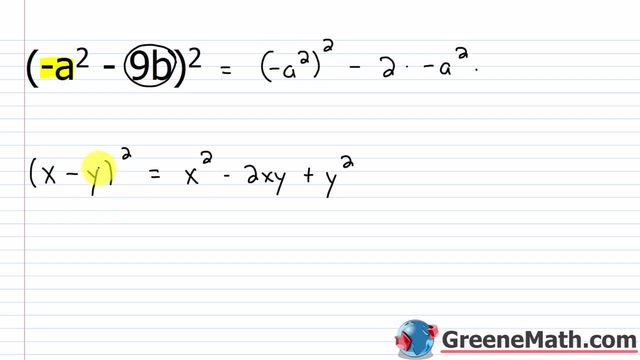 I just take whatever's in that position, Just like here. I just take y, right, I don't put negative y in, So you've got to follow that formula to the t. I'm going to put 9b in there. 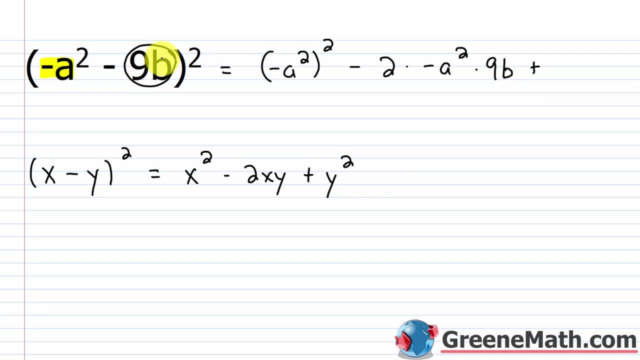 And then last I'm going to have, plus this guy: 9b squared. So 9b squared. All right, let's erase this. OK, And let's erase this. All right, let's crank this out. So, if I have negative, a squared squared. 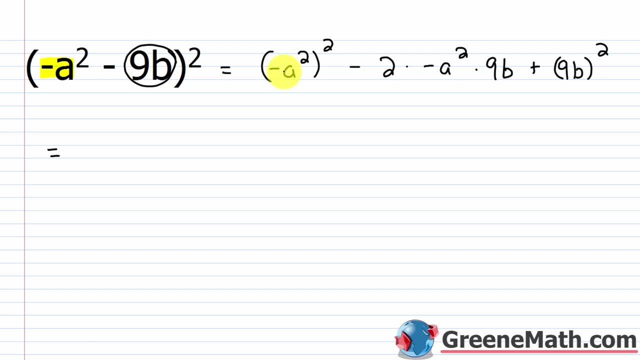 I know this is basically negative 1 squared, That would be 1.. So this would be positive And then a squared squared. Keep a the same And multiply exponents 2 times 2 is 4.. Then next we would look at: we have negative 2 times negative, a squared times 9b. 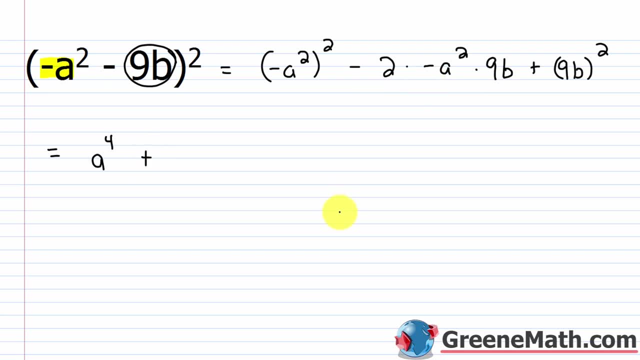 Negative times. negative is positive, So I know this would be plus. And we think about 2 times 9,, that's 18.. And we'd have a squared times b, So a squared b. Then, lastly, we have 9b. 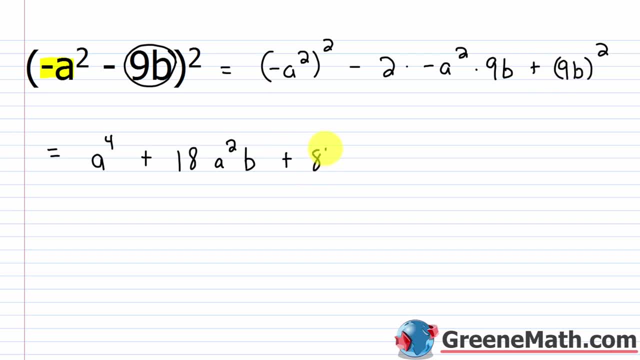 That amount squared, So plus 9 squared is 81.. b squared is just b squared. So we end up with a to the fourth power plus 18, a squared, b plus 81, b squared. So just something you want to look out for is when they throw these signs at you. 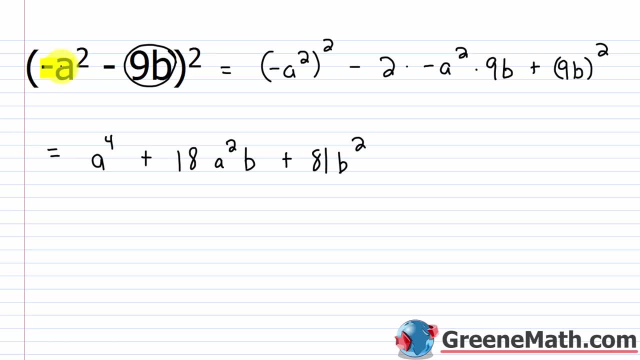 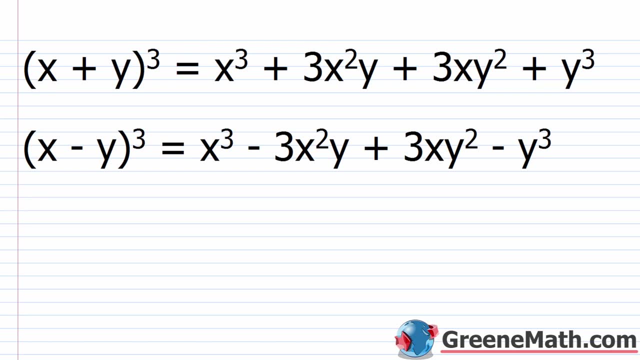 If you put a negative out in front of that first term, OK, Pay close attention to that, All right. So the last thing I want to talk about is when you have a binomial cubed, So this one's a little bit more tedious. 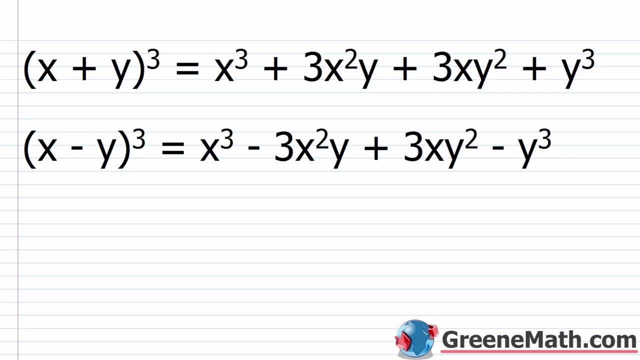 But this one will also save you more time, Because as you multiply more terms, it gets more tedious, It becomes more easy to make a mistake And it takes you longer to do the process. So memorizing these will have the greatest value for you. 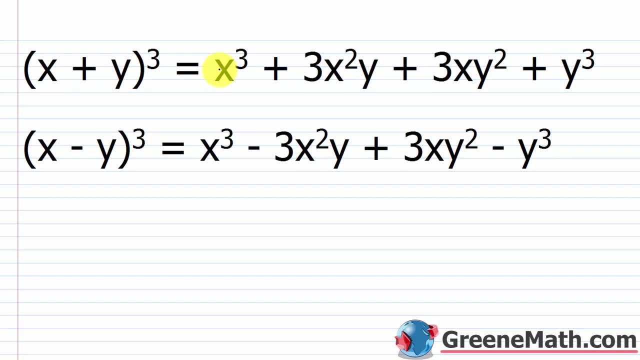 So if I have the quantity x plus y and it's cubed, I get x cubed plus 3x squared y plus 3xy squared plus y cubed. Now if I have the quantity x minus y and that's cubed, it's the same thing, only the second. 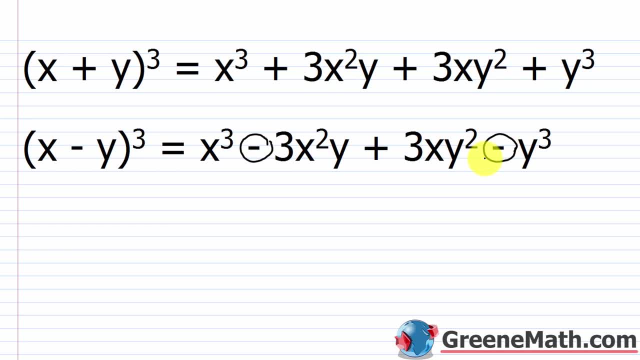 position and the fourth position have minus signs in front. So x cubed minus 3x squared y plus 3xy squared minus y cubed. Now, in terms of memorizing this guy, it's a little bit more complicated. I always just remember that I have x. 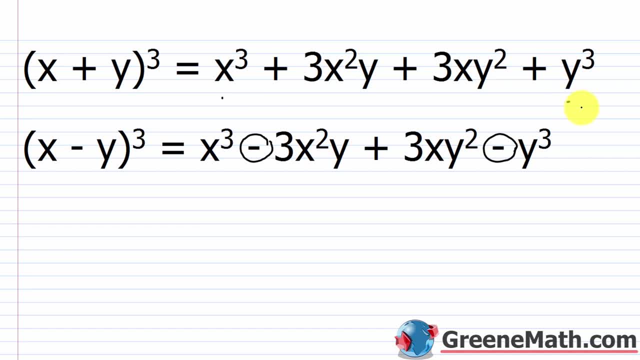 cubed and y cubed at the beginning and at the end. So that's easy. Then I know I'm multiplying with a three in each of the two middle terms, Just like when we looked at the square of a binomial, I knew I was multiplying by a two. 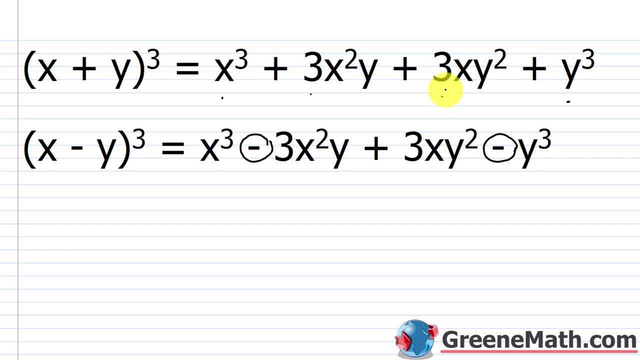 And that was two times the first term times the second term. That's pretty easy to remember. Here. you have a square involved in each case, So it's kind of goes back and forth. But if you just remember that the first term is squared in one case, the second term is squared in the other case. 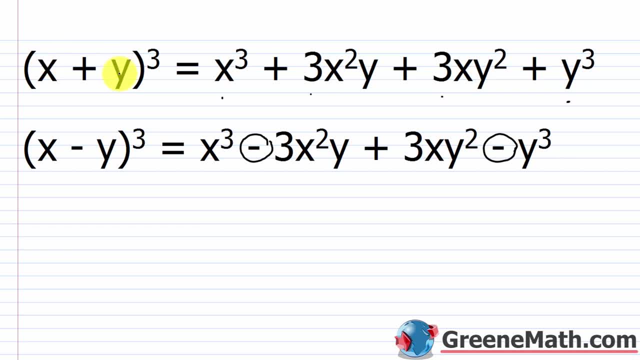 So it's three times one of these squared times, one of these to the first power in each case. In the first case, we have three times the first term, squared times the second term. Then we have three times the first term, which is not squared times the second term, which is squared. 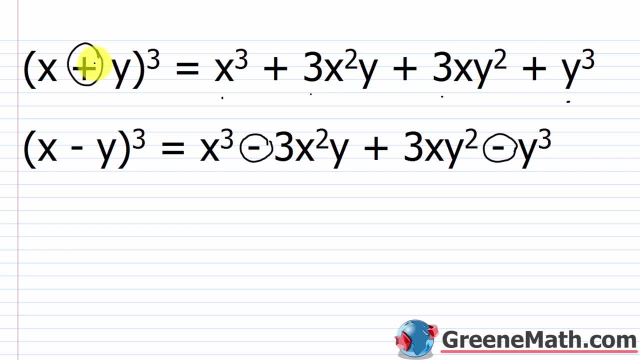 Okay, And then the only difference between this one where we have a plus and this one we have a minus is the minus sign in front of the second and fourth terms. And again, I know this seems daunting, but You work 10 or 15 problems looking at this and representing it and going back and forth. 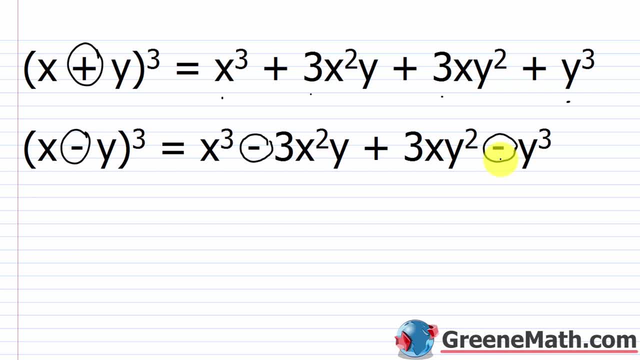 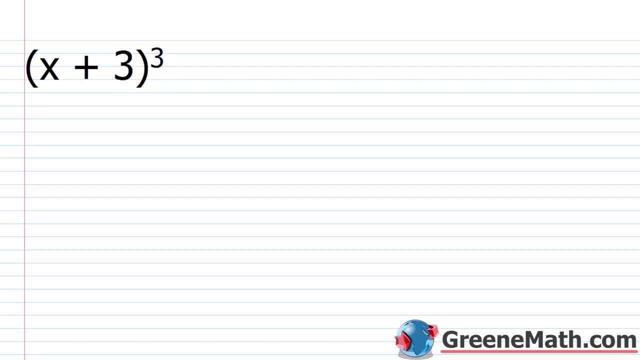 You're going to have this down and it's going to save you a tremendous amount of time. All right, Let's look at an easy one to start. So let's suppose we had X plus three, that quantity cubed. Well, what's going to happen again if I put the quantity X plus Y cubed? what is this? 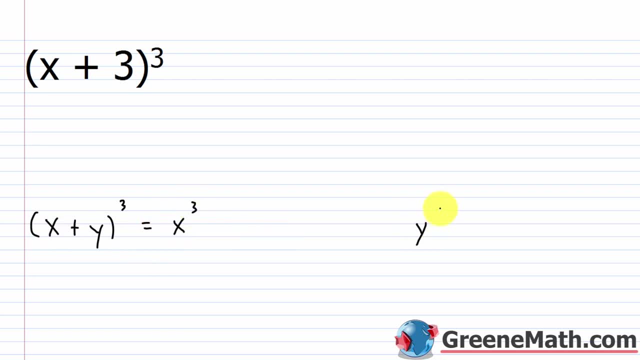 Again, I know I have X cubed in the beginning and I know I have Y cubed at the end. I know that I have two terms, I know that I have two terms in the middle and I know it involves multiplication with three right. 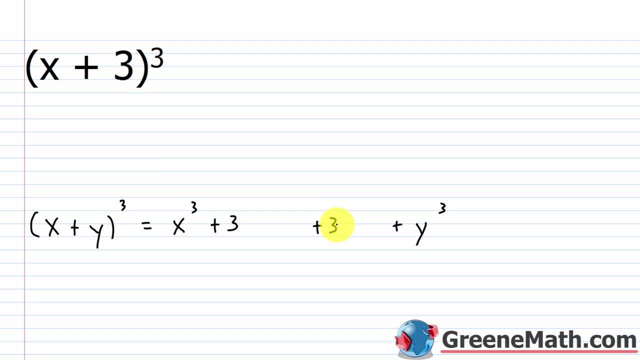 So three and then three. Now, all you need to remember is that I'm multiplying by the two terms here. One of them is squared in each case, One of them is not. So if I start out by just saying: okay, X would be squared. 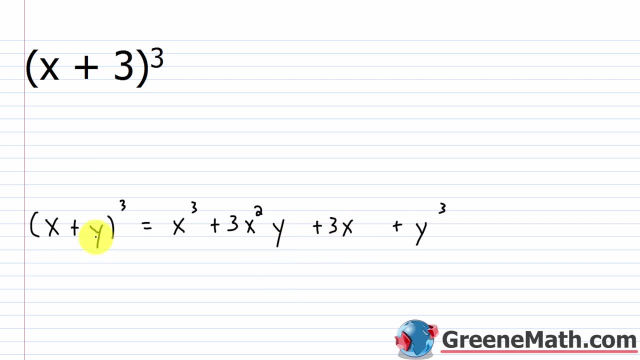 Y is not, Then if I say, okay now, X will not be squared, Y will be squared, Boom, Got my answer. It's just that simple. So I'm just going to apply that technique here. So I have X plus three. 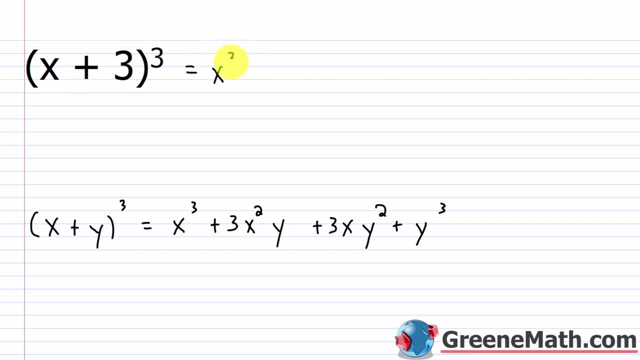 That quantity. So the first guy is cubed, So X cubed. The last guy is cubed, So three cubed. Let me put that all the way down here. Now I'm going to have three multiplying by these two terms for the two middle terms. 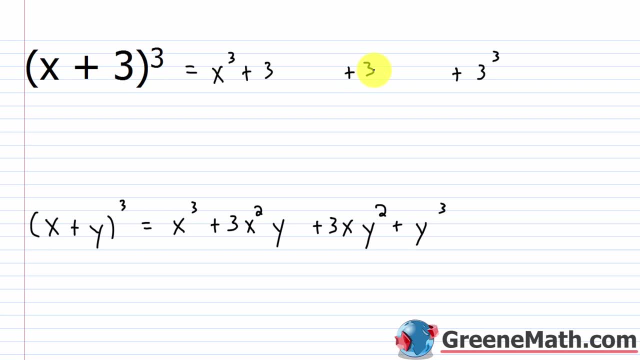 So let me put that in there, And then in each case, one of them will be squared, One of them will not. So I'm going to square X: Three will not be squared. Then I'm going to square three: X will not be squared. 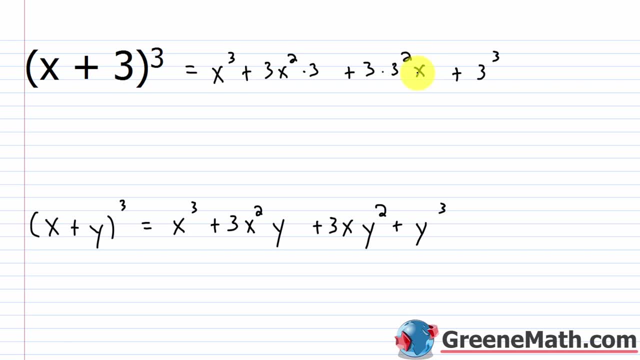 And that's it. I've got my answer. It's really really that simple, All right. So let's erase this And you can see how much quicker this would be versus kind of expanding this out into X plus three. that quantity times X plus three, that quantity times X plus three, that quantity. 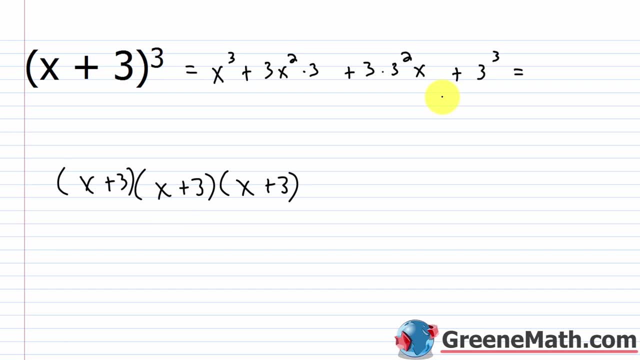 This will take a while. Okay, Doing it this way is going to be much, much quicker for you. All right, So we have X cubed to start. Then we have three X cubed, X squared times three. Three times three is nine. 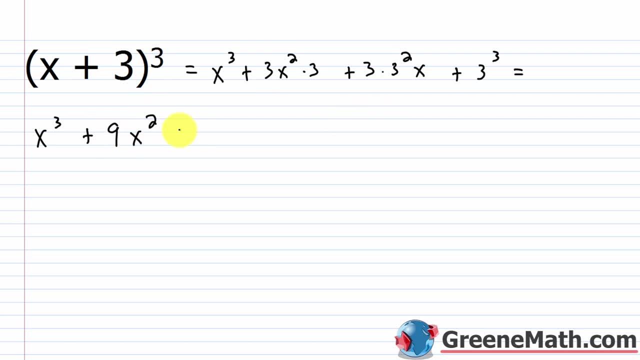 So plus nine X squared, Then we'd have plus. You have three times three squared times X. So three squared is nine. Nine times three is 27.. 27 times X is just 27 X. And then lastly, plus three cubed, which is 27.. 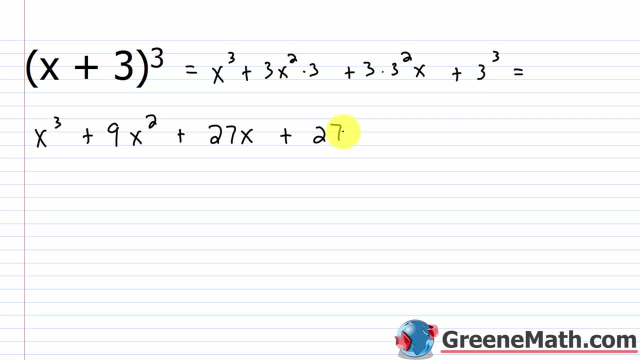 So we get X cubed plus nine, X squared plus 27, X plus 27.. All right, Let's look at another easy one. So we have the quantity X minus two and that's cubed. So can we do this without writing out the pattern? 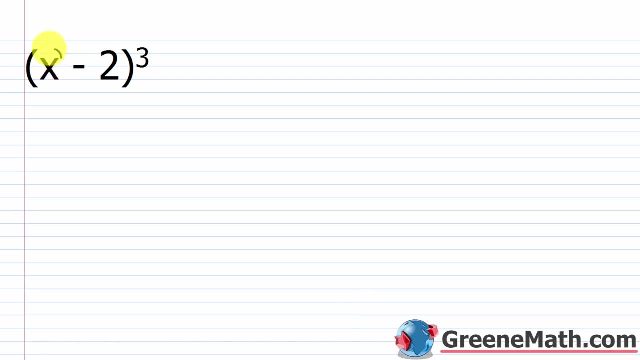 I think that we can. So again, I know that I want this first thing- cubed, So X cubed. I know that I want this last thing, cubed, So two cubed, And I'm going to go ahead and write that as eight. 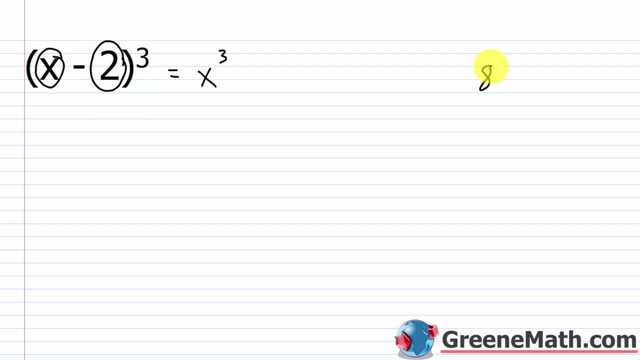 We know two cubed is eight, So let me write that all the way down here. Now, as far as signs go, I know in front of the second term and the final term or the fourth term, I have minus signs, So there'll be something here. 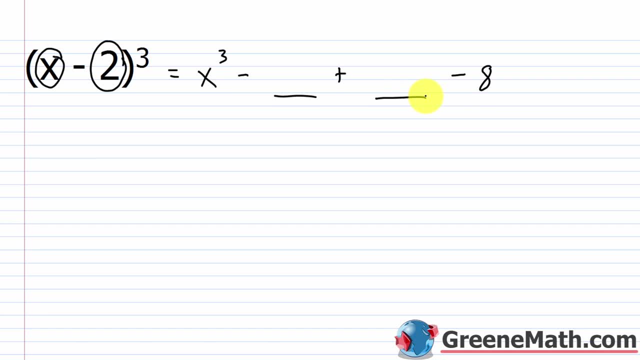 There'll be a plus sign And then something here. Now, what do we remember? We remember that these two middle terms here have a three, that's leading. So let's put a three in each case, And I'm multiplying by each term here. 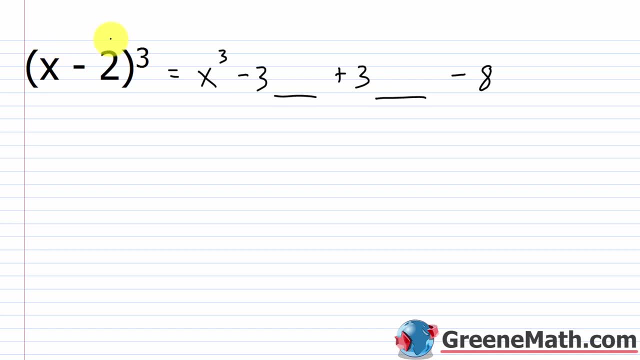 It's just that one of them will be squared in each case. One will not. So we start out with X being squared and then two not being squared. Then we'll have X not being squared and two being squared. Boom And we're done. 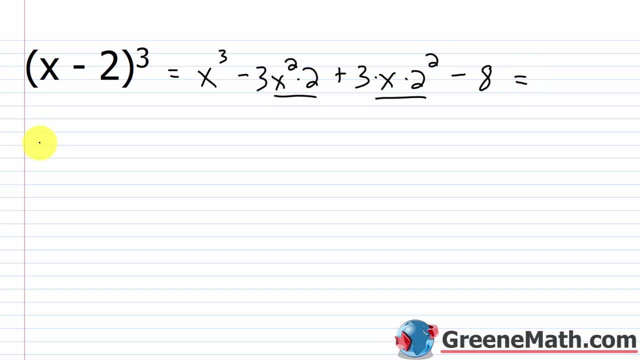 It's just that easy. Okay, So we have X cubed. minus three times two is six. Six times X squared is six X squared. And then plus two squared is four. Four times three is 12.. 12 times X is 12 X. 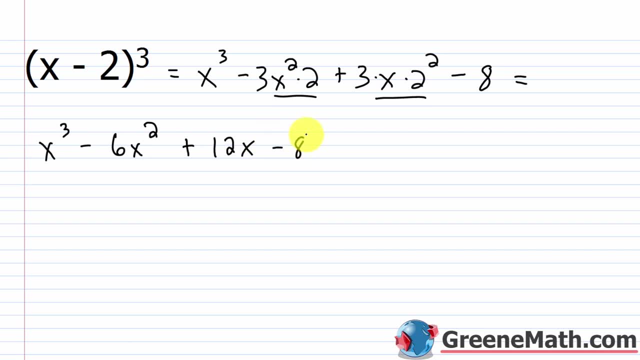 And then minus eight, We're done. Okay, And again, think about how much time that saved us And we had to go through and do the pattern. I could just kind of do this mentally and have this answer in a few seconds. 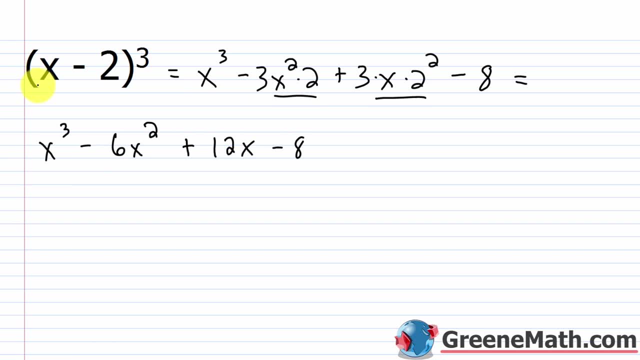 Okay, And you'll be able to do that too. So if you're on a standardized test and it asks you for the quantity X minus two cubed, you can get that answer in a few seconds and kind of move on versus somebody that's got to take out scratch paper. you know, expand this into the quantity X. 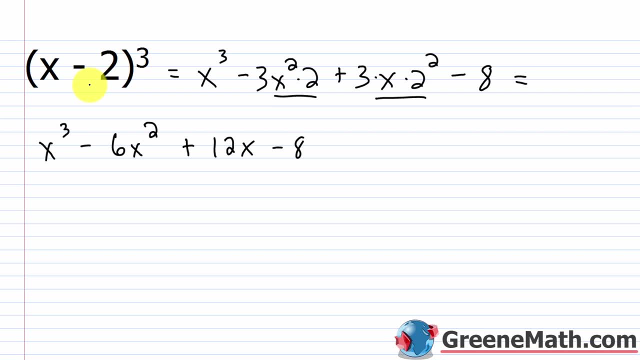 minus two times X minus two times X minus two, They might be there for a full minute. Okay, So you're ahead of somebody by a full minute. Now, that's time you can apply to a more difficult problem, Right? So let's look at one final one of these. 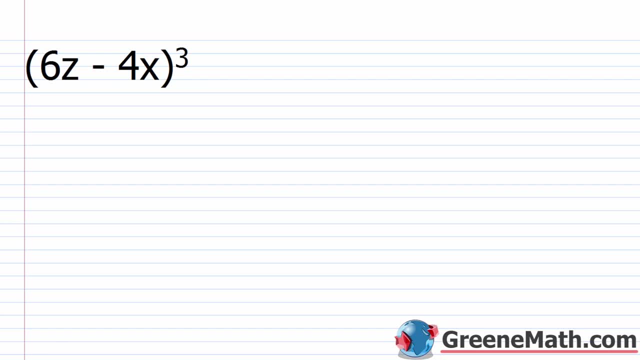 It looks a little bit more complicated, but really it's not. We have the quantity six Z minus four X, and this is cubed. So again, what am I going to do? I know that I want this first guy cubed. 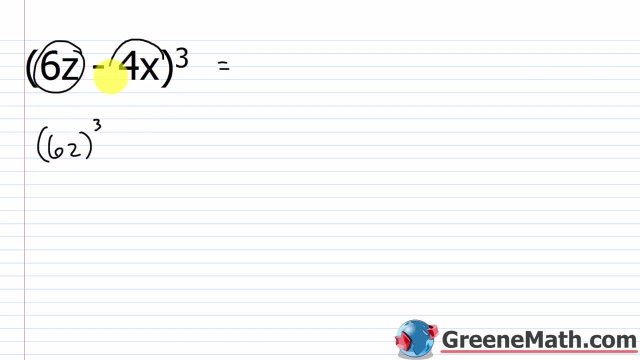 So six Z: I know I want that cubed. I know I want this last guy cubed. So let me throw this all the way down here and say we have four X and that's cubed. I know that I'll have a minus sign in front of the second guy and the fourth guy. 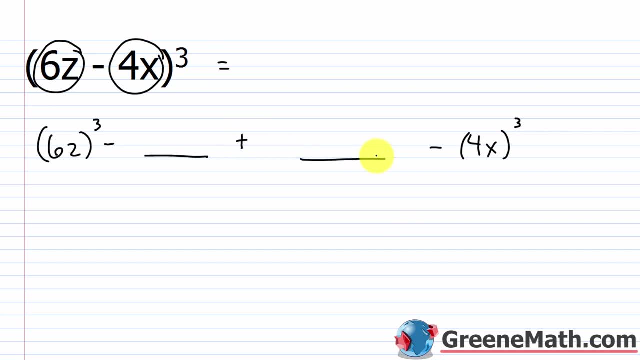 So I'll have something here, I'll have a plus sign and something here. We kind of move that down a little bit. So it's more even and I know that I'm going to have a three that's multiplying the two middle terms. 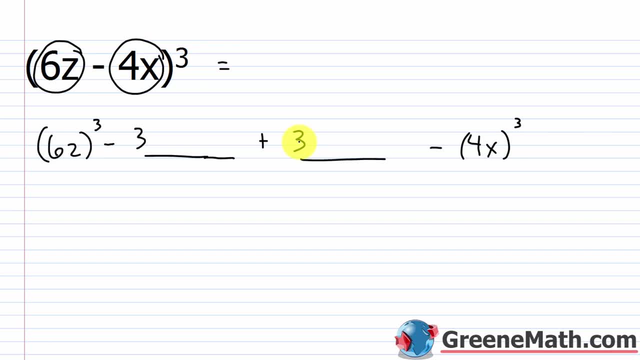 Now, in each case, one of the terms when we talk about the middle terms will be squared, One of them will not. So I'm going to multiply this by. I'll have six Z squared times four X. In this case, I'll have six Z not squared and four X as squared. 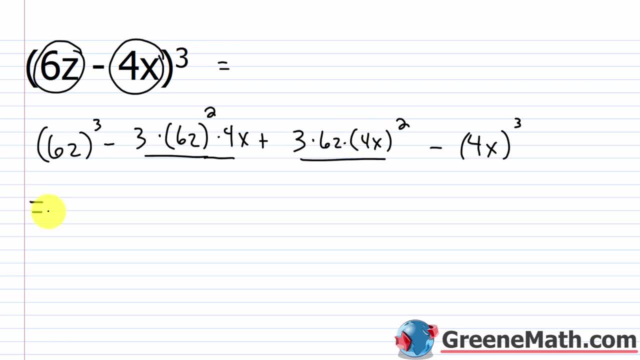 And that's it. Now we just have to go through and do some calculations. So six Z cubed, the six is cubed. Six times six is 36.. 36. Six times six is 216.. Z cubed is just Z cubed. 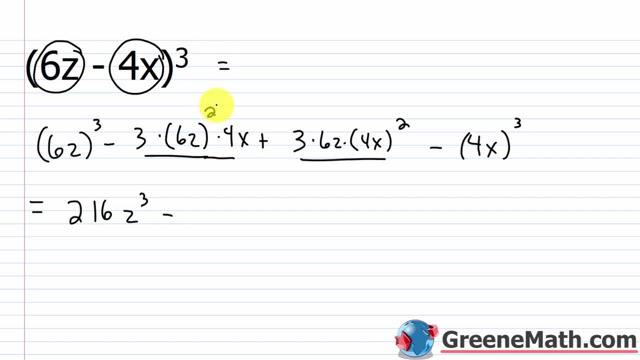 Then we'd have minus, So then we'd have six Z squared, which is basically going to be 36 Z squared, And 36 times three is 108.. Then if I multiply by four, I get 432.. So minus 432, you would have X and then Z squared. 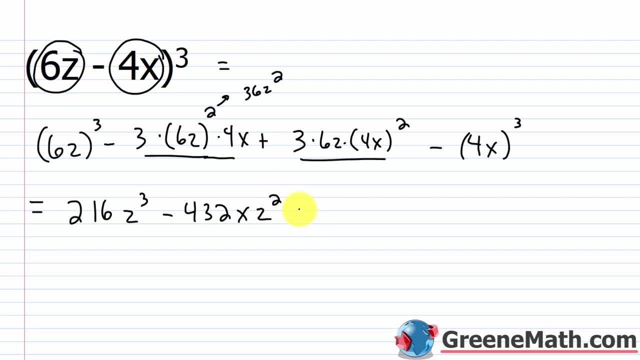 So X- Z squared, And then plus You have three times six, Z times four, X, That amount squared. So this right here would be four squared times X squared. We know four squared is 16.. So let's write 16 X squared for that. 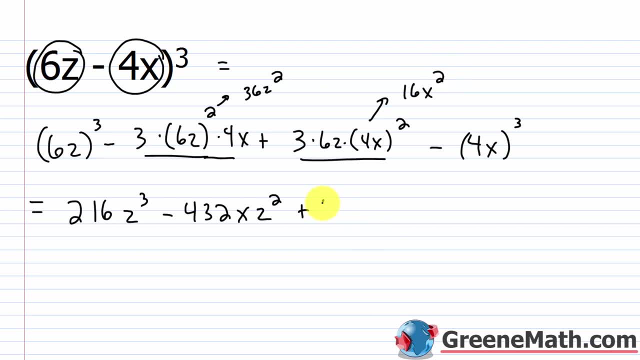 So three times six is 18.. Then 18 times 16 would be 288.. And you'd have X squared Z. Then, lastly, you have minus, You have four X cubed. Four cubed is 64. And then X cubed is just X cubed. 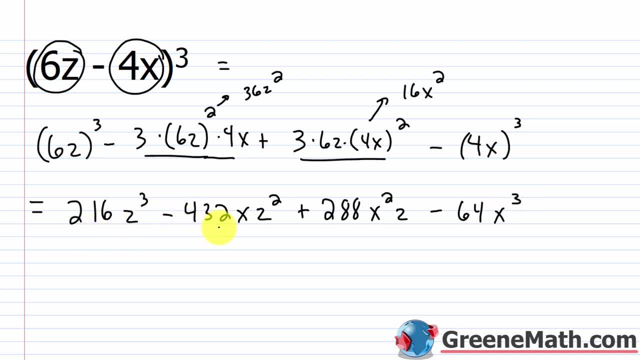 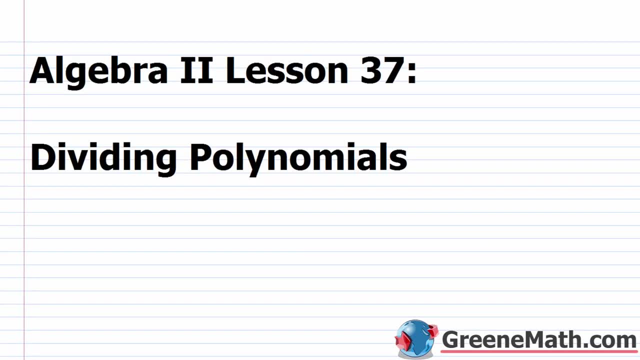 So we have 216 Z cubed minus 432 X Z squared, And then we'd have 16 X squared Plus 288 X squared Z minus 64 X cubed. Hello and welcome to Algebra 2, Lesson 37.. In this video, we're going to learn about dividing polynomials. 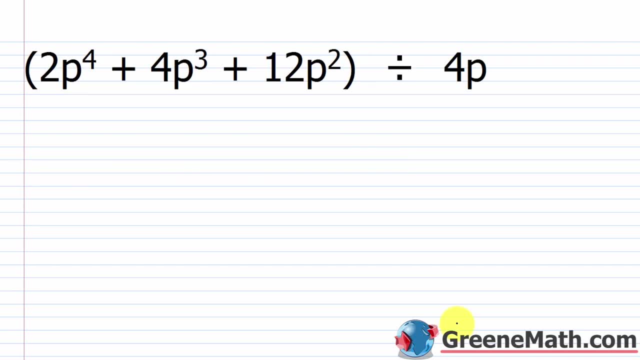 So again, for most of you, if you've taken an Algebra 1 course, you already know how to divide polynomials And this lesson is nothing more than a review for you. If you haven't taken Algebra 1, or if you kind of struggle through Algebra 1,, 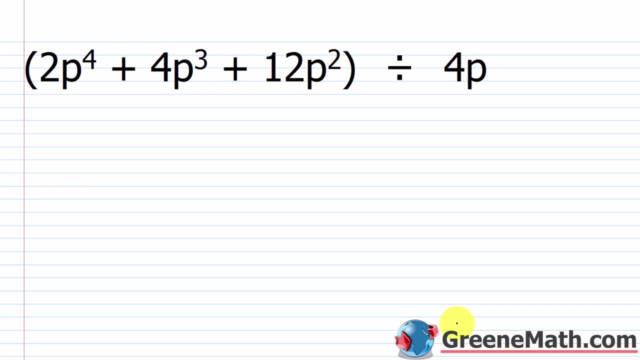 you can pick this topic up from this lesson. I'm going to kind of start at the very beginning. I'm going to go a little quicker than I did in Algebra 1.. But still, you can pick it up from this lesson. The first thing I want to talk about is the easiest scenario. 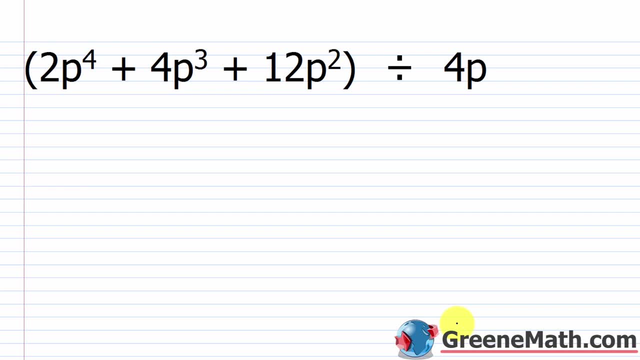 If we divide a polynomial which is not a monomial meaning- it's not a single term only- by a monomial meaning, it is a single term only. So that's what we have here. in this first example, Let's say I had 2P to the fourth power plus 4P cubed plus 12P squared. 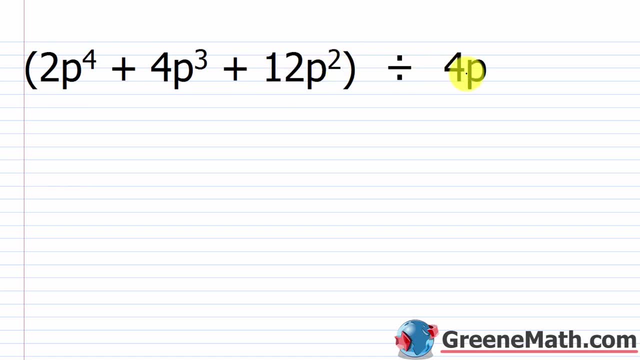 And it's divided by 4P. The very first thing you want to do is write this as a fraction, So let's take this as the numerator of the fraction. So 2P to the fourth power plus 4P cubed, plus 12P squared. 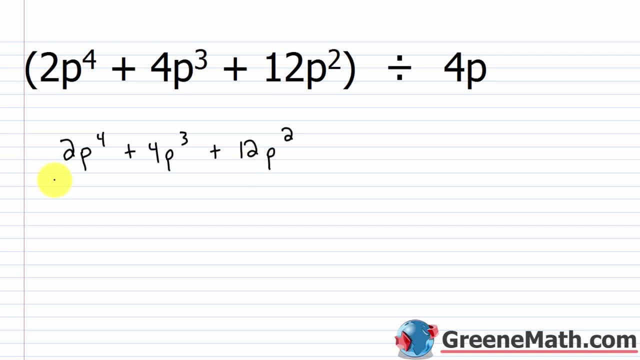 That's going to be my numerator, That's my dividend. Then I'm going to put this over my denominator or my divisor of 4P. Now we know from our work with fractions that we could split this up and write this as each term. 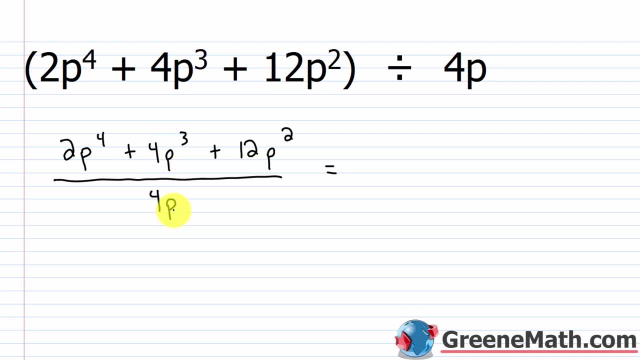 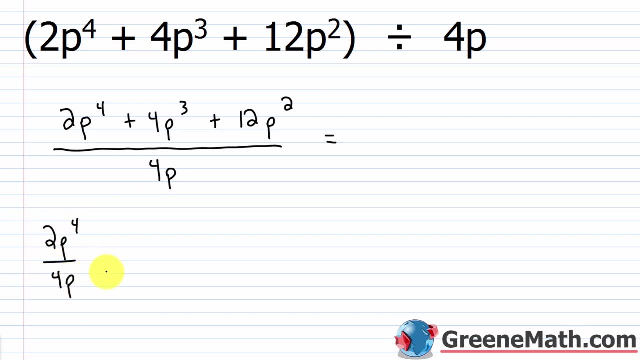 of the polynomial and the numerator over that monomial from the denominator. In other words, I can say this is 2P to the fourth, power over 4P plus 4P, cubed over 4P plus 12P squared over 4P. 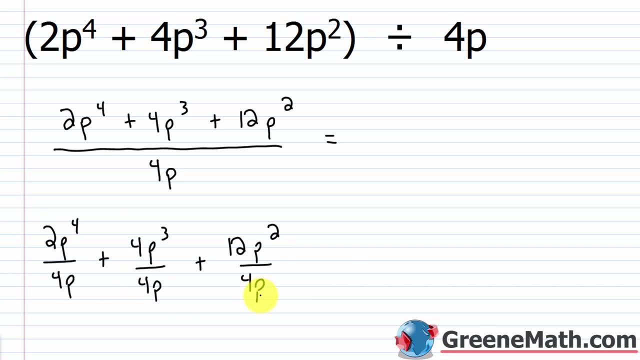 And you can just think about taking this format right, There's a common denominator and, going to this format, It's no different than if I had something like 6 over 2.. I could say this is 6 over 2 plus, let's say 4 over 2, right. 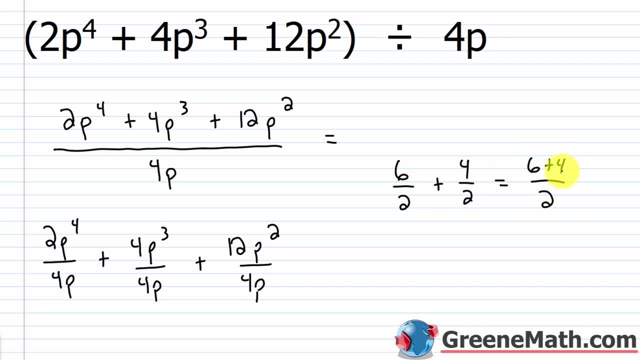 I could say this is 6 plus 4 over 2.. 6 plus 4 is, of course, 10.. 10 over 2 is 5, right, So it's the same thing. All right, so let's erase this. 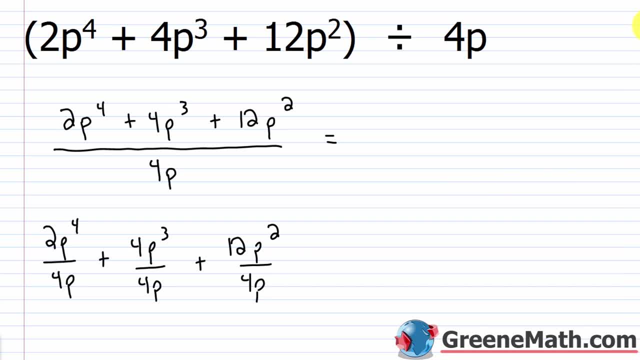 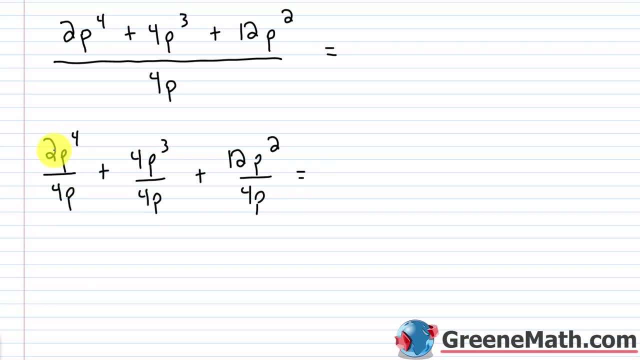 And let's focus on this. So what I want to do is attack this problem piece by piece, And what I mean by that is I'm going to start right here, all the way on the left, And I'm going to say 2 over 4.. 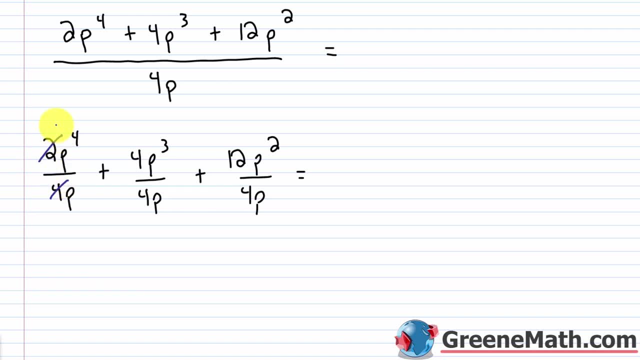 Well, I know it's not going to be the same thing. I know 4 divided by 2 is 2. So I can cancel this with this. I'll put a 1 here and a 2 here. P to the fourth power over P to the first power. 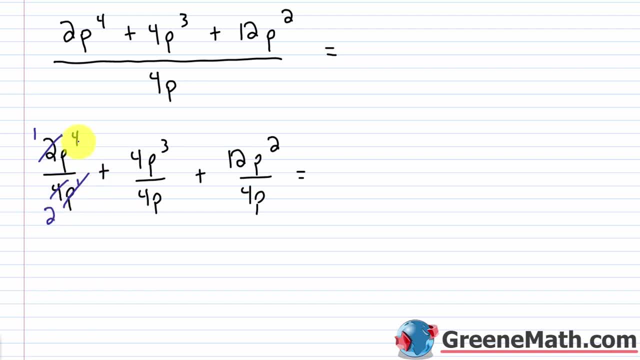 I can cancel one factor of P, So this would cancel and this will become a 3.. Then over here I go to this part. next I have 4P cubed over 4P. The 4s will cancel P. cubed over P to the first power is P squared. 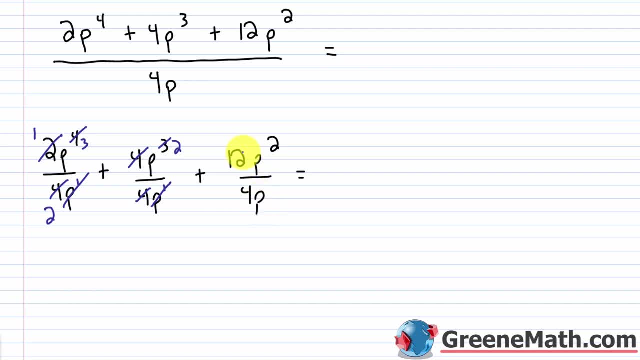 Then I go to this part. I have 12P squared over 4P, 12 divided by 4. It's 3.. P squared over P is P to the first power. So just look at what is remaining to write our answer. 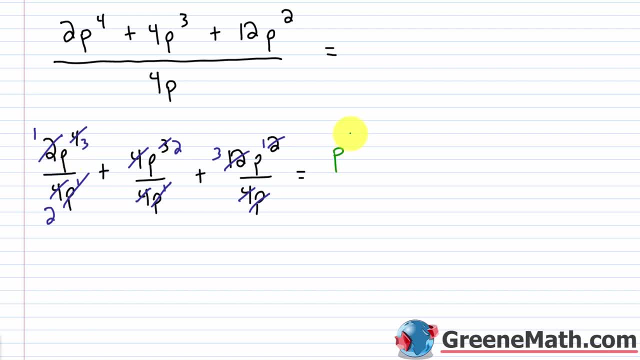 We have 1P cubed or just P cubed, This is over 2.. Then plus, we have P squared, Then plus, Next we have 3P, We have 3P, All right, So P cubed over 2, plus P squared, plus 3P. 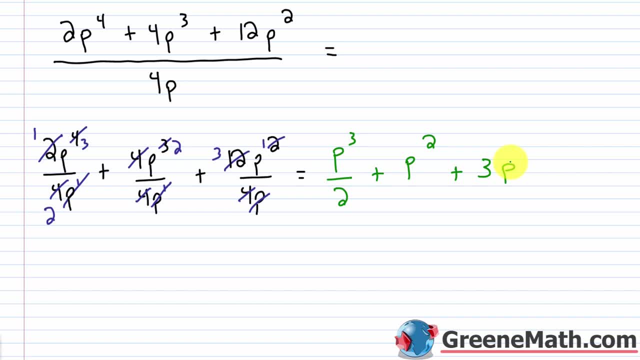 So that's your answer. Now we know, with division, we can check our answer. Whatever our quotient is in this case, this is the quotient. This is the quotient. We could multiply this by the divisor and we would get the dividend back. 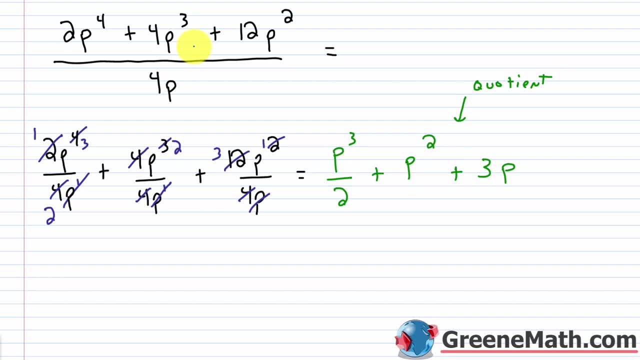 And I'm not going to do that in the interest of time, but you could pause the video and you could multiply 4P by each term here and you would come back to 2P, to the fourth power, plus 4P cubed, plus 12P squared. 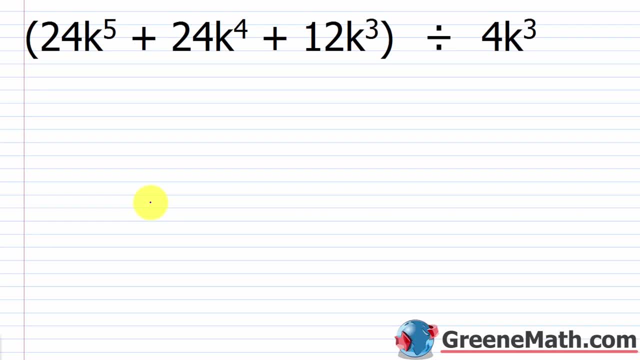 All right, Let's take a look at one more like this. So let's say we have 24K to the fifth power plus 24K to the fourth power plus 12K cubed, And this is divided by 4K cubed. 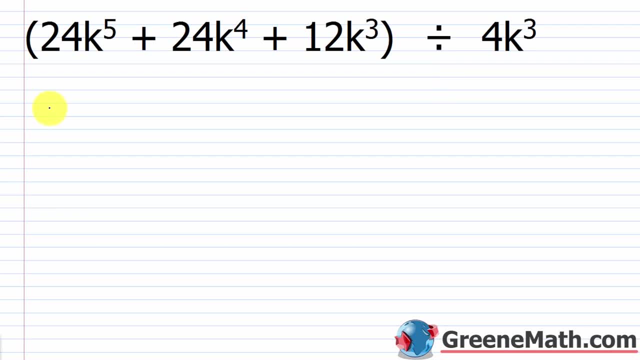 Again, the first thing I would do in this scenario is write this as a fraction. So my dividend goes in the numerator. So 24K to the fifth power plus 24K to the fourth power plus 12K cubed, Then this is over. 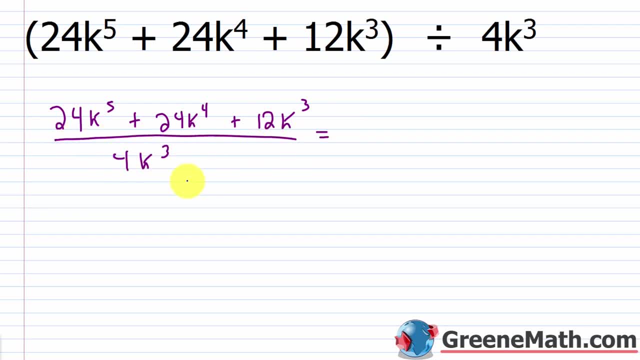 24K cubed. And then I'm going to split this up. So I'm going to say, okay, I have 24K to the fifth power over 4K cubed, Then plus 24K to the fourth power over 4K cubed. 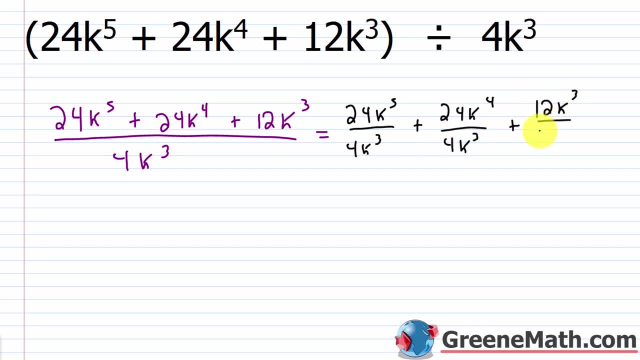 Then plus 12K cubed over 4K cubed, All right. So now what I want to do is just go through and simplify. Let me put equals here: 24 divided by 4 is 6.. K to the fifth. power over K cubed would be K squared. 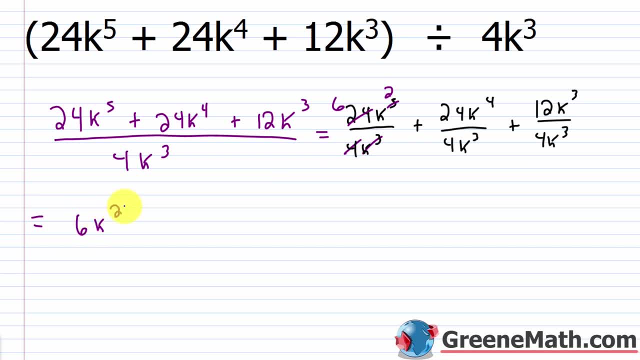 So the first result here would be 6K squared. Then I'm going to put plus For the next scenario. again, I have 24 over 4.. That's 6.. I have K to the fourth power over K cubed. 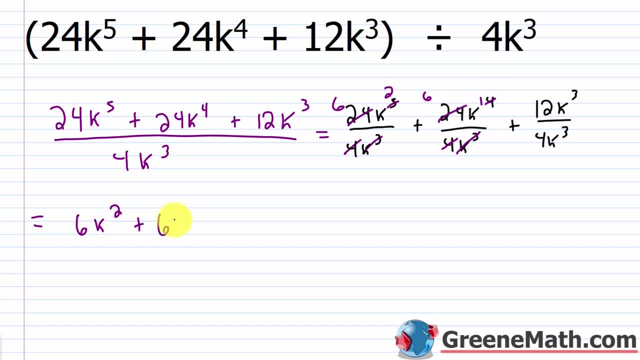 So this cancels and I have K to the first power, So I have plus 6K. Then, lastly, I have 12 over 4, which we know is 3.. And then K cubed over K cubed is 1.. 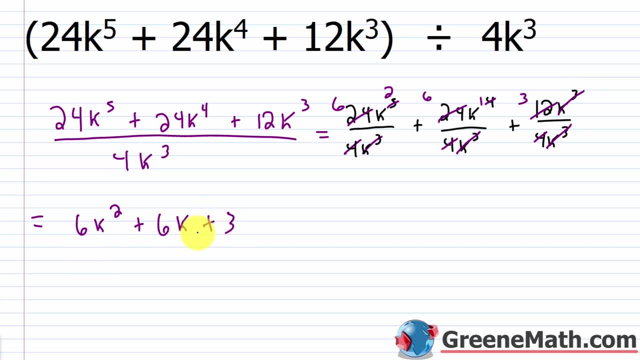 So basically that's just plus 3 there. So your answer is okay. I have 24K to the fourth power over 4K cubed. So the answer or your quotient here is 6K squared plus 6K plus 3.. 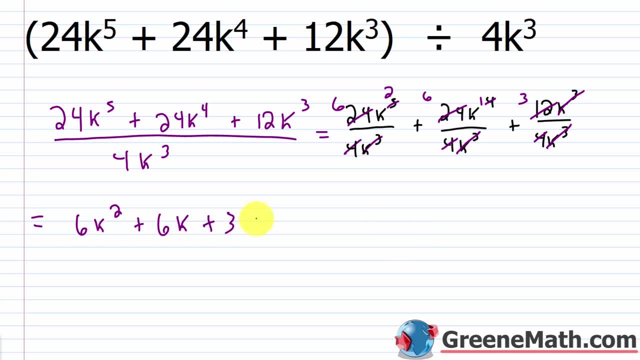 Now again, this is division, So if you wanted to check it, you could take your quotient right here, multiply it by your divisor, which is 4K cubed, and you will get your dividend back, which is 24K to the fifth power plus 24K to the fourth power plus 12K cubed. 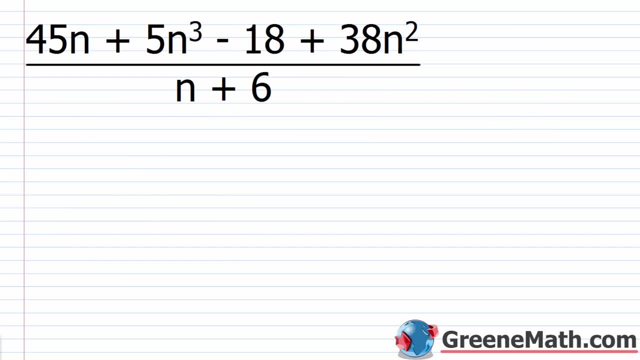 Okay. So that's the very easy scenario that we first deal with when we're dividing polynomials. In an Algebra 1 course, you usually have a section that's just devoted to that, learning how to start out with dividing a polynomial by a monomial. 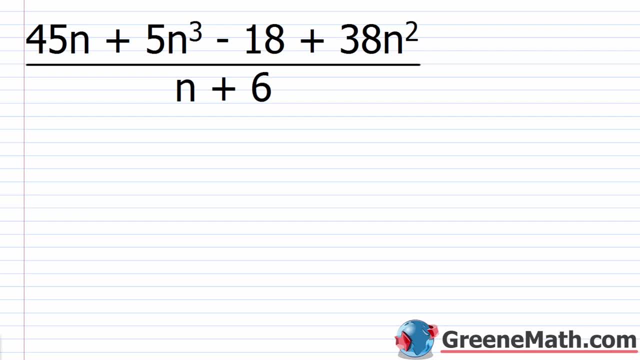 Then you kind of move on and you look at two different other sections. The first thing is dividing polynomials with long division, So you divide a polynomial by another polynomial that is not a monomial. And then you also hit another section where you do this and you have missing terms involved. 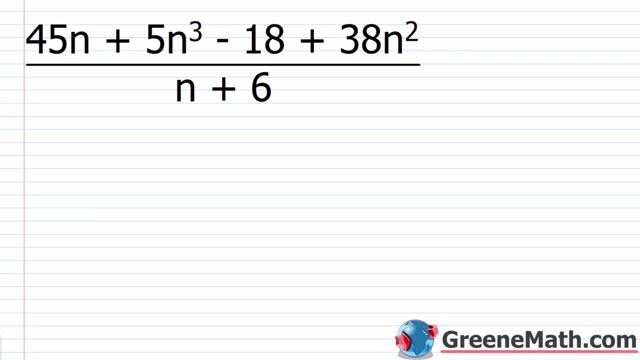 So the process is similar to when we divided whole numbers. So if you were good at long division you might want to do a few problems just to kind of get your brain re-acclimated to that. We're pretty much going to do the same thing here. 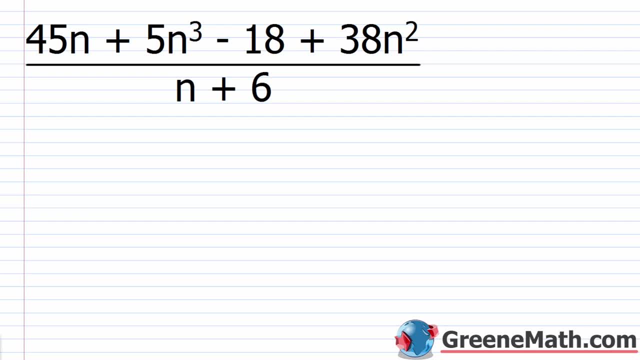 The first step to this is to write each polynomial in standard form, And if you have a polynomial that's missing any powers for your variable, you want to put zero as a placeholder. So I would start out with this example here: 45N plus 5N, cubed minus 18 plus 38N, squared over N plus six. 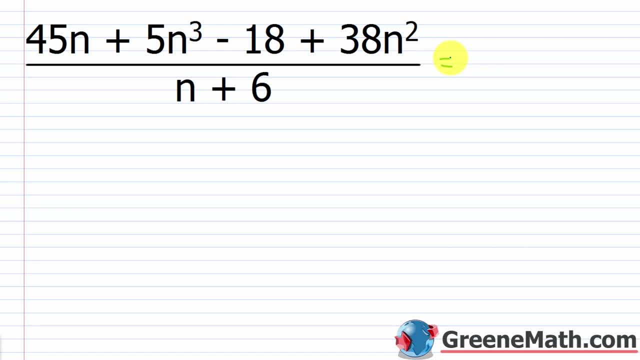 So for right now, I'm just going to keep it in this format, but I'm going to write everything in standard form. So remember, I want the highest power on N all the way to the left. So that's going to be 5N cubed. 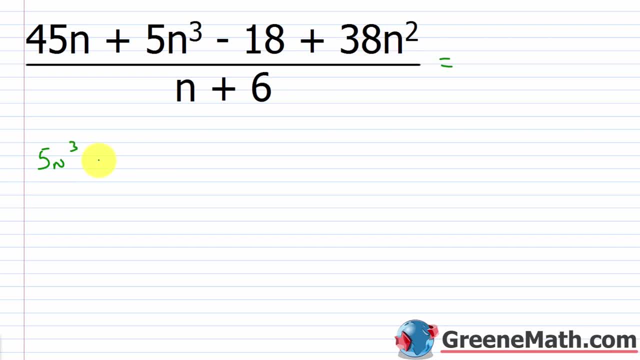 So 5N cubed, Then next I'm looking for squared, So plus 38N squared. Then I'm looking for first power, So plus 45N. Then I'm looking for a constant, or you could say N to the power of zero. 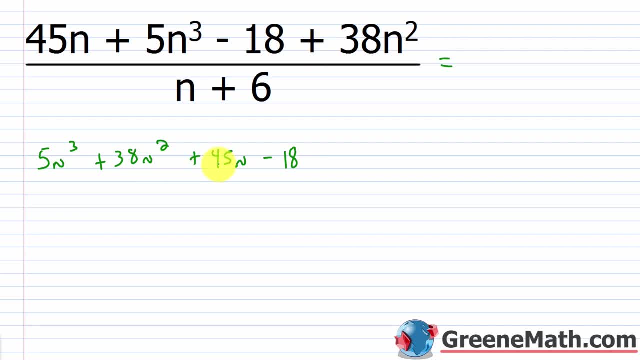 So minus 18.. Okay, So that's in standard form. Now I'm not missing any powers for my variable. I have a third power, second power, first power and basically power of zero, So I don't need to write zero as the coefficient for any missing powers. 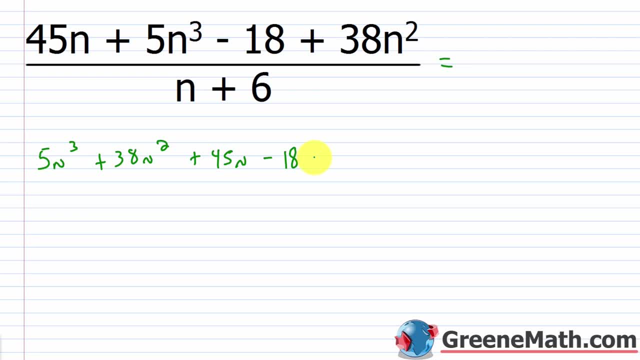 but we'll see an example of that in a little while. So then this is over. We have N plus six, So that's already in standard form. I have N to the first power plus my constant, which is six. All right, 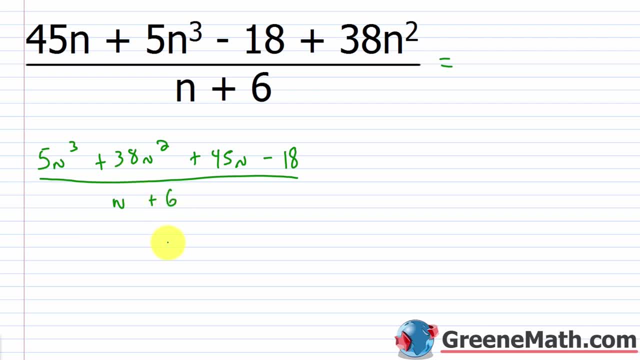 Let me erase this. We don't need that Now. what we want to do, What we want to do is we want to write our problem in long division format, So you'll recall if you had something like, let's say, I'm going to do this on a different page. 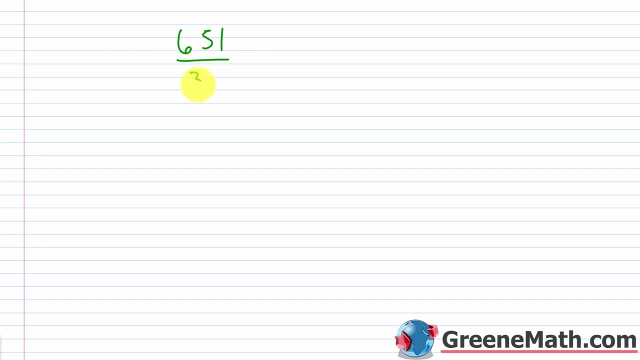 651 divided by, let's say, 31,. something like that. Well, we could write this as 651 divided by 31, like that. Or we could also write this as 651 divided by 31, like that. This is just long division format. 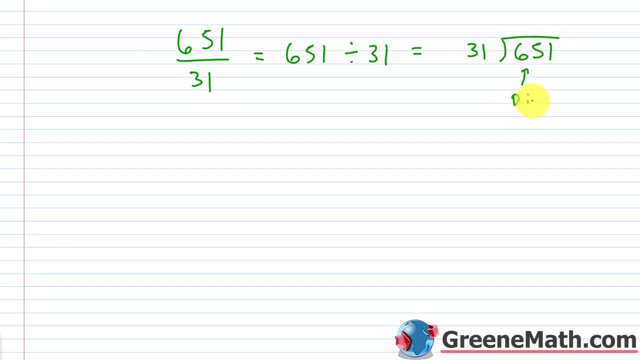 The 651 is the dividend. This is the dividend And the 31 is the divisor. Okay, The divisor. So the divisor goes to the left of our symbol and the dividend goes underneath. So we're going to do the same thing. 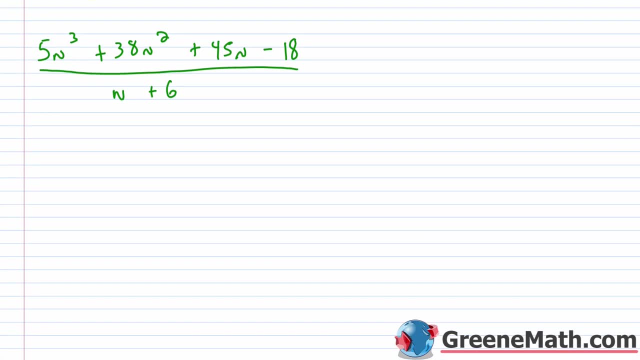 And what I'm going to do. let me just kind of scroll down a little bit So we have some room. I'm going to take the dividend here and let me label that This is the dividend And I'm going to put it under the. 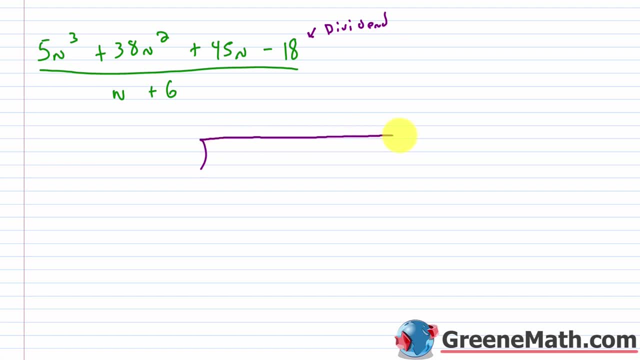 Long division symbol. So I have my long division symbol and I'm going to write my dividend underneath. So five and cubed plus 38, and squared plus 45 and minus 18.. And then my divisor. my divisor goes out to the left. 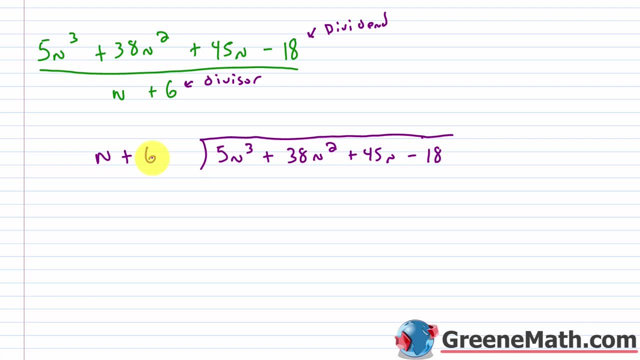 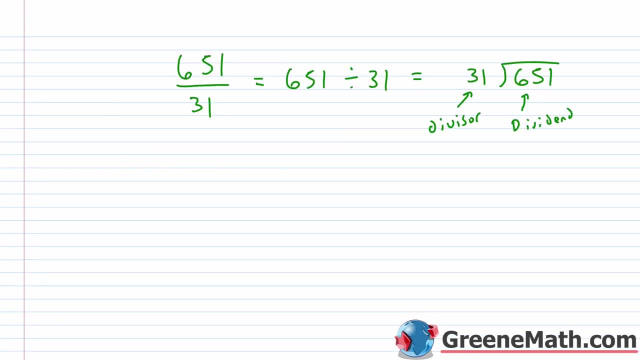 So, and plus six, Okay, So the process for long division with whole numbers, as you'll recall. let me kind of go back down to this Example. I'm going to erase this real fast. It's going to give us some room. 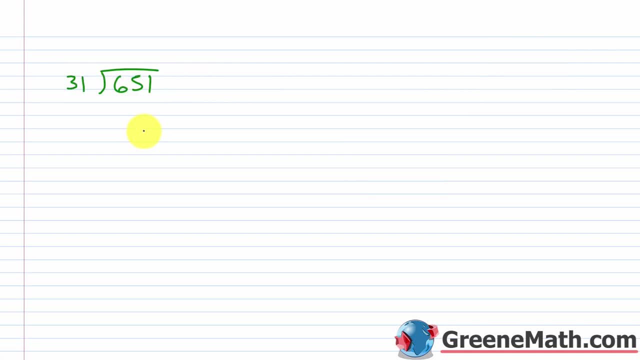 And let me just scooch this to the left. We use this D, M, S, B, R to remember this. This is divide, multiply, subtract, bring down and then repeat or remainder. A lot of teachers will remind you of the family unit and use a little trick to remind you of it. 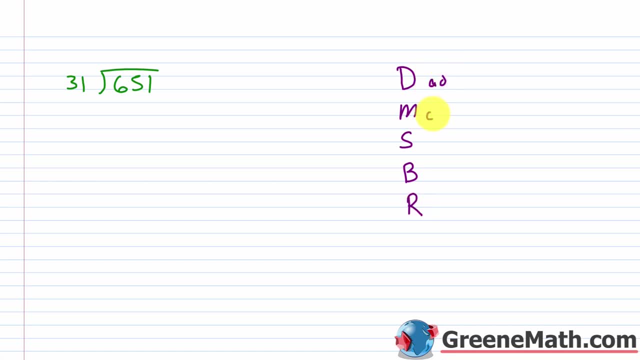 They'll say dad, mom, sister, brother, and then Rover, right. So the family unit: a mom and a dad, a brother and a sister and then a family dog. So I would start out with this first step of division. 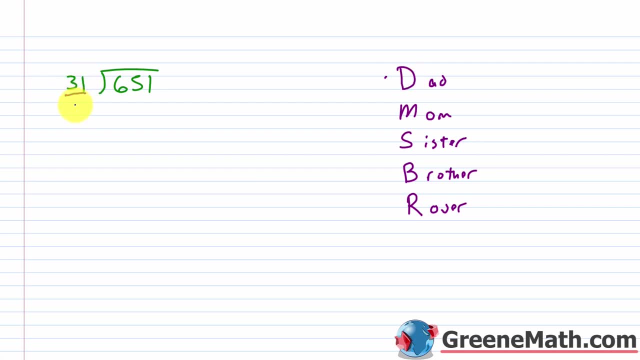 I would say how many times this 31,, which is your divisor, go into, and I'd start out with this piece by piece. So let's say, how many times does it go into six? Well, it doesn't, So you could put a zero here. 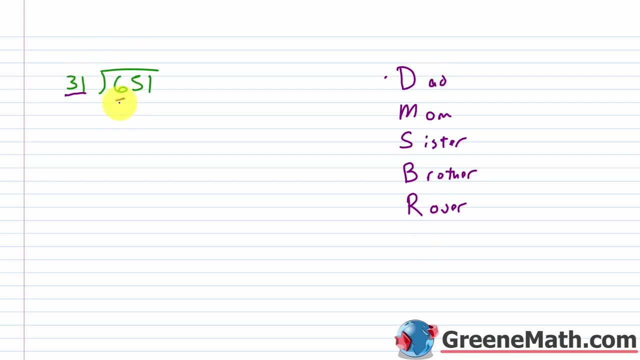 Zero here And you could go through kind of the steps there or you could just make it a little quicker and you could expand this and say: how many times does 31 go into 65?? Well, 31 goes into 65 twice. 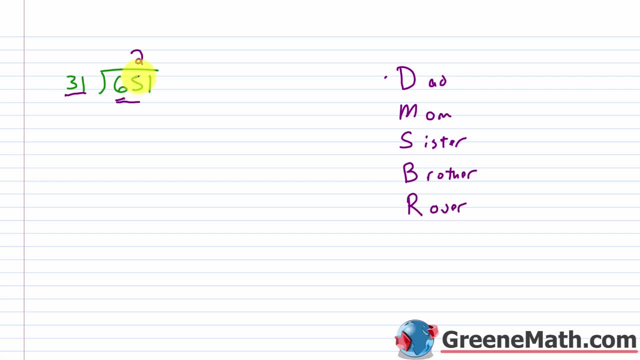 So I would put a two over the five, right, Because that five is in the tens place. that two stands for 20. And then I would multiply: Okay, That mom step. So two times 31 is 62. Then I would subtract the sister step: 65 minus 62 is three. 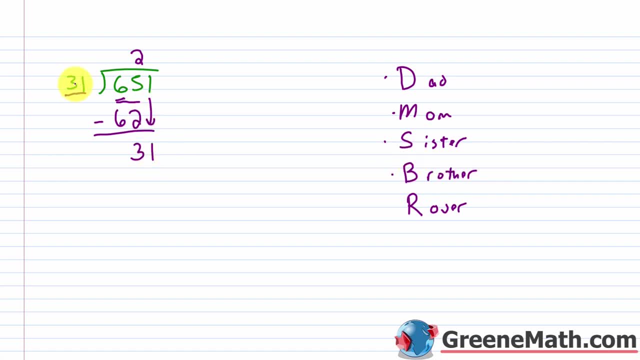 Then I would bring down the brother step, So this one would come down, then I would repeat or remainder, which is the Rover step. In this case we're going to repeat the process. So we're coming all the way back up here and we're going to divide again. 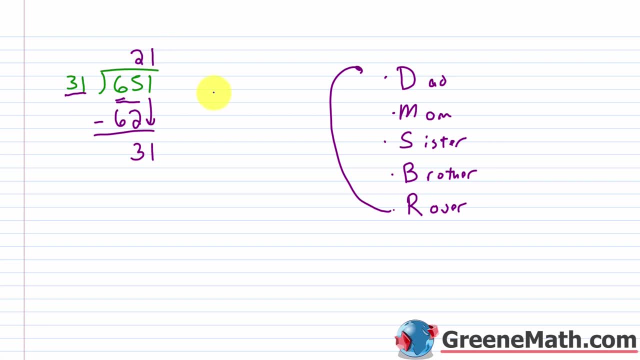 So now 31 goes into 31 one time. We're going to multiply one times. 31 is 31.. We're going to subtract: 31 minus 31 is zero. There's nothing to bring down. We're at the step where we repeat which we're not going to do, or we'd have a remainder, and there is no remaining. 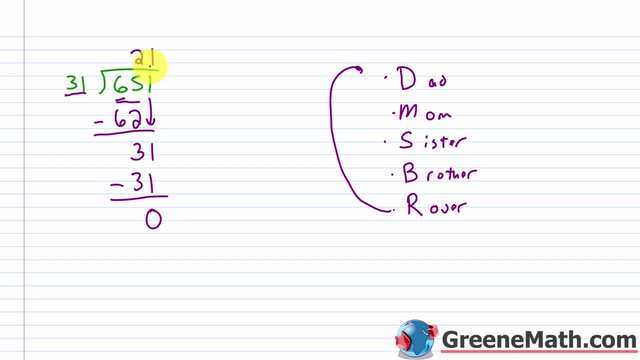 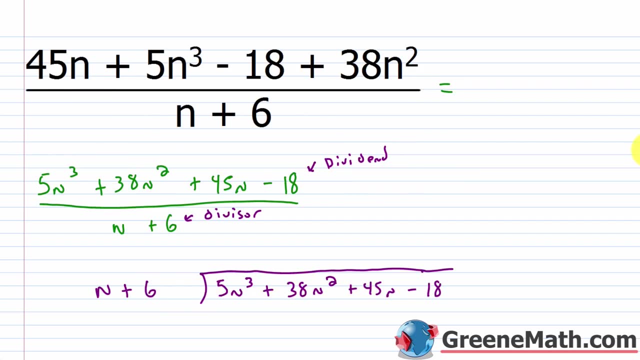 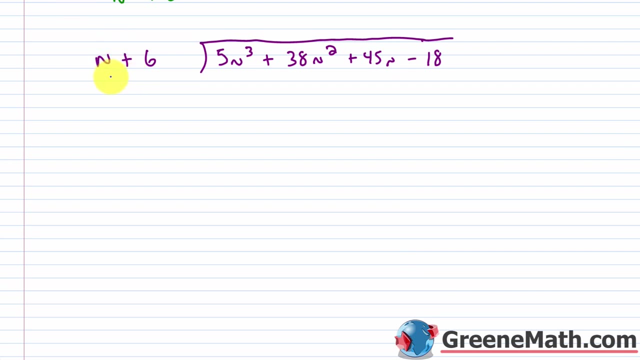 So we saw that 651 divided by 31 is 21.. Okay, So it's basically the same thing When we start doing our division here. the only real difference here is I'm only going to think about leading terms. So when I look at my divisor here, I'm going to start by saying leading term into leading term. 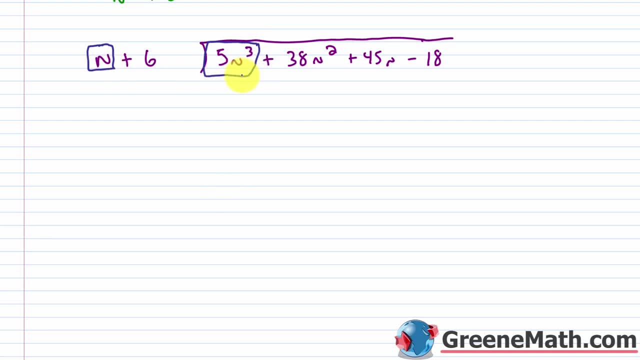 So the question would be: how many times does N go into five N cubed? That's my first Step, or my division step. So I would say: five N cubed over N equals what. Well, I know five's not going anywhere. 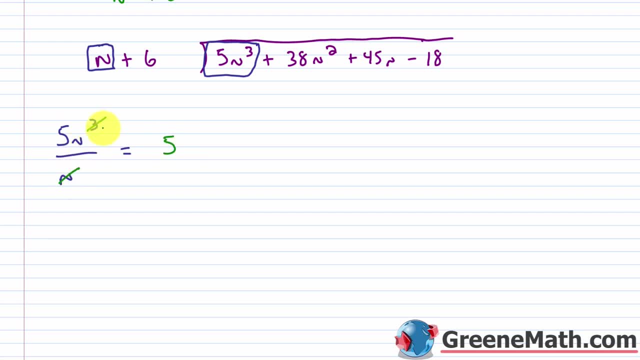 It's just N cubed over N, So this would cancel with this and be this right: N cubed over N would be N squared, So you'd have five times N squared. Now a lot of students make this mistake and they'll just say, okay, well, I'll just put five N squared here and we'll just keep going. 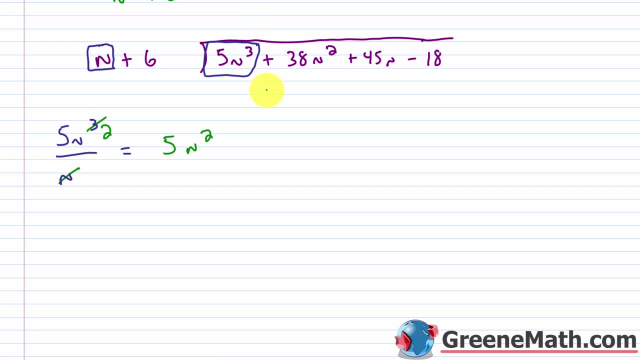 You don't want to do that. This has Place value, just like what we just saw. This is the place to put N cubed right here in this column. This is the place for N squared. This is the place for N. This is the place for your constants. 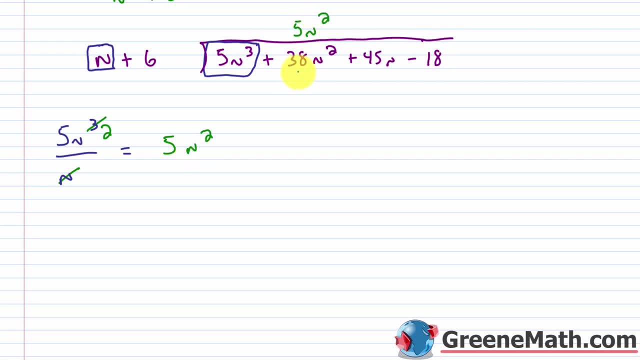 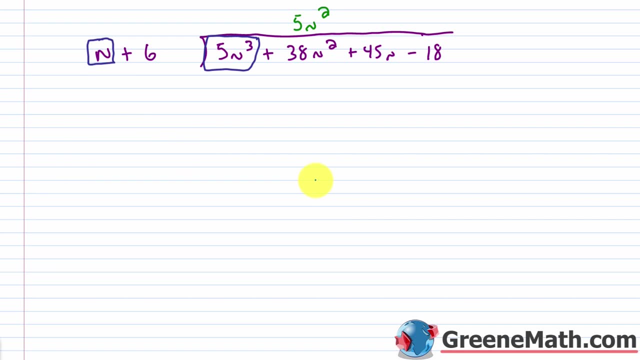 So my answer is five N squared. So I want to put it here over the 38 N squared. Once we've kind of done that first step, the next thing is to multiply. Now when I multiply, I multiply by everything. So I multiply this result here by this whole. 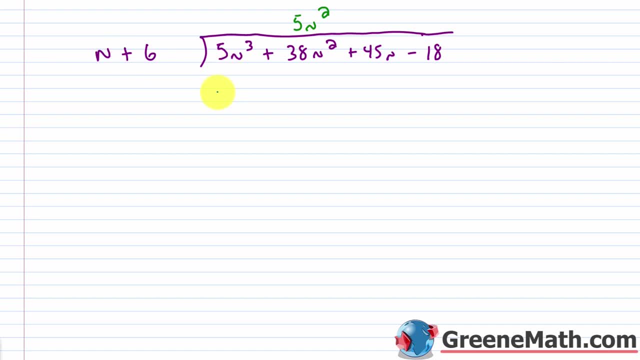 Thing here. So five N squared times N would be five N cubed. Then five N squared times six would be 30 N squared. Now I want to subtract away, And the main mistake here is that people just put a subtraction symbol out in front and they start subtracting. 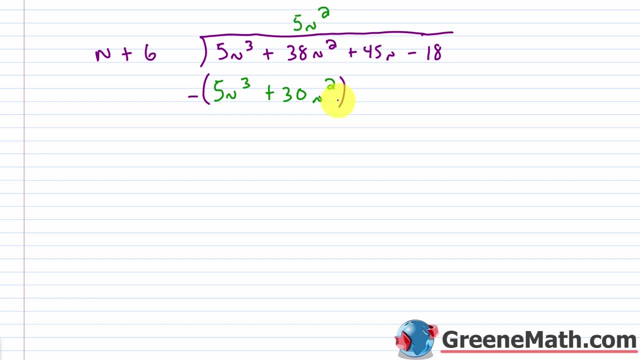 So really I want parentheses around this And what I can do is I can just change the sign of each term that's being subtracted away and add. So a quick trick to this would just be OK. I list everything and then I just change the size. 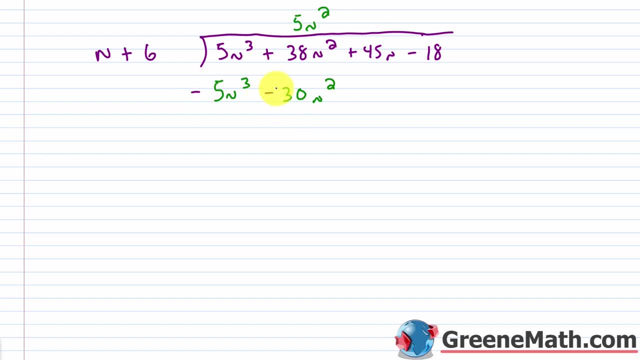 So this would be negative and then this would be negative. Now I can just add: So I put a little bar here and I'll add five N cubed minus five N cubed at zero. Thirty eight N squared minus 30 N squared is eight N squared. 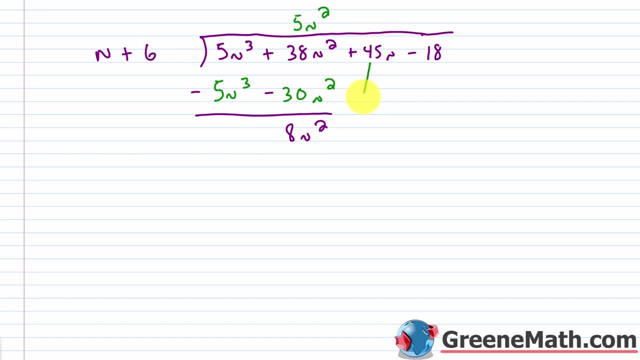 Now my next step is to bring down. So the next term is here. I'll bring that down. So plus 45 N. And then I just repeat the process Again. I'm going to go leading term into leading term, So N goes into eight N squared. 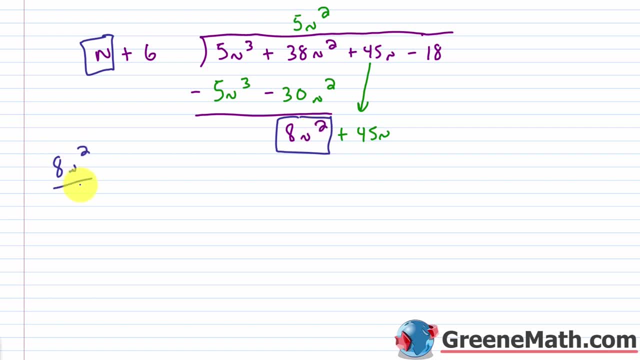 And again, if you want to write it out on the side, eight N squared over N to figure that out, that's fine. Most of you at this point can kind of do that in your head. OK, we know that eight N squared divided by N would simply be eight N. 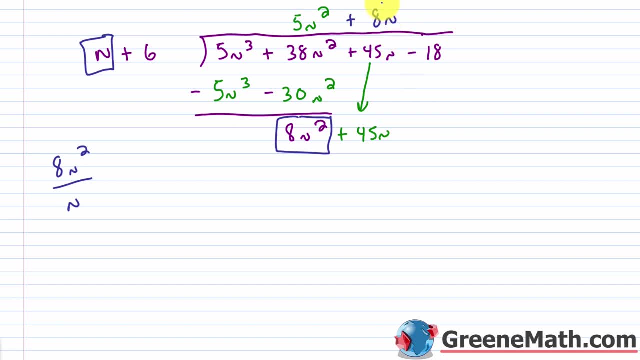 So we would write plus eight N And look how it lines up with the place value. This is where 45 N to the first power is. This is where eight N To the first power. So again, we're maintaining our place value there. 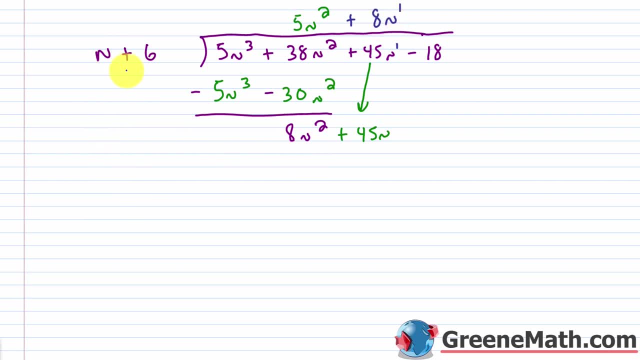 Now the next thing is again to multiply. So eight N times N is eight N squared, And then eight N times six is 48 N. Now I can put a minus sign out in front and put my parentheses Again. the shortcut to this is just to remember. I'm going to change the sign of everything there and I'm going to add: 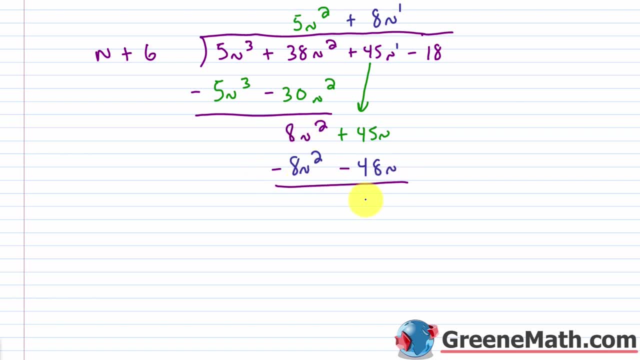 So eight N squared minus eight N squared would be zero, And then 45 N. 45 N minus 48 N would be negative three N Again I want to bring down as my next step. So I'm going to bring down that negative 18.. 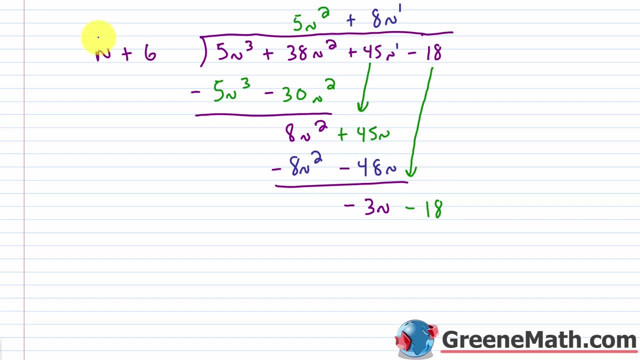 And then once again, for the last time, I'm going to go leading term into leading term. OK, so N goes into negative three N. How many times You're asking yourself the question: what is negative three N divided by N? 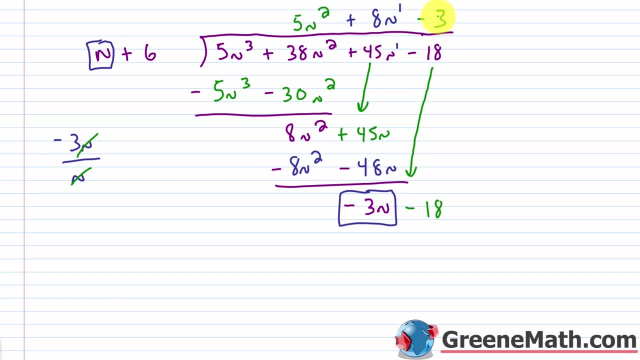 So N cancels with N And I'm just going to get negative three. So now I multiply. So what is negative three times N, That's negative three N. What is negative three times six, That is negative 18.. Now you have the same thing here and here. 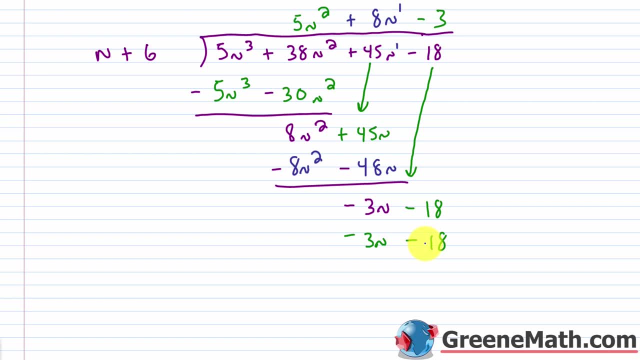 If I subtract the same thing away, I'm going to get zero Right. And you can prove that to yourself again by changing the sign of everything and adding: So this becomes plus, and this becomes plus, And we add Negative three N plus three N is zero. 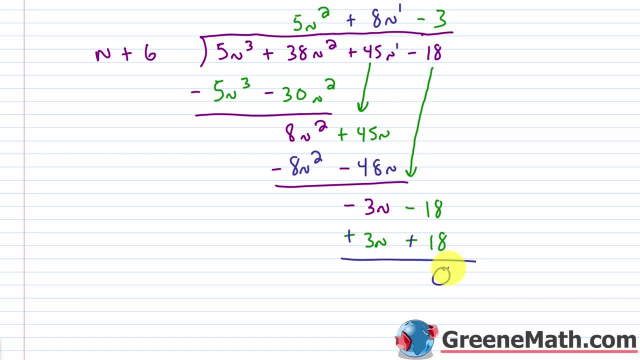 Negative: 18 plus 18 is zero. So there's no remainder. OK, and sometimes you have a remainder, Sometimes you don't. OK, in this case we don't. So our quotient is five N squared plus eight N minus three. 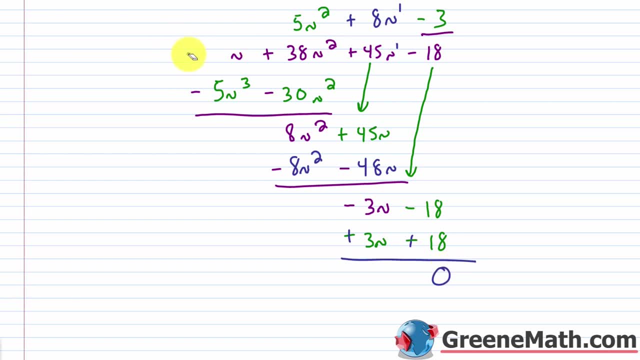 So I just want to show you something. Let me erase kind of everything except for the answer, And I'm going to prove to you that this works. Let me kind of scroll up a little bit. I'll just kind of drag this up here. 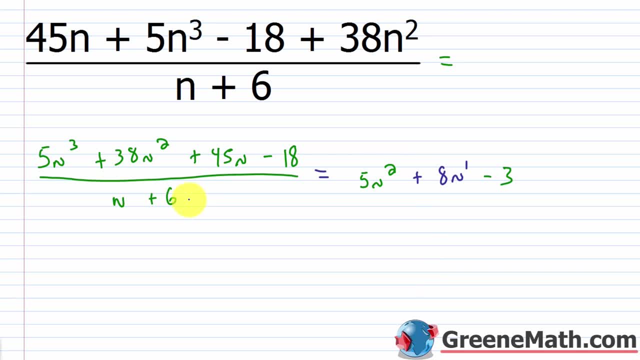 All right. So what I want to do in order to prove this? I want to multiply the divisor by the quotient That should give me the dividend back, if I got the correct answer. This is how you can always guard against mistakes. It's just like if I had six divided by three, and this equals two. 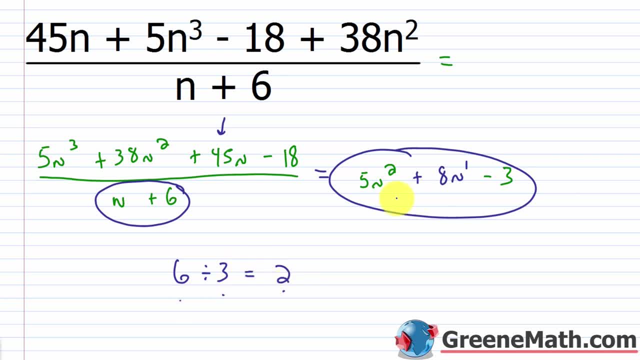 I could say: two times three gives me six. It's the same thing. I'm saying: five N squared plus eight N minus three times the quantity N plus six is going to give me five N cubed plus 38 N squared plus 45 N minus 18.. 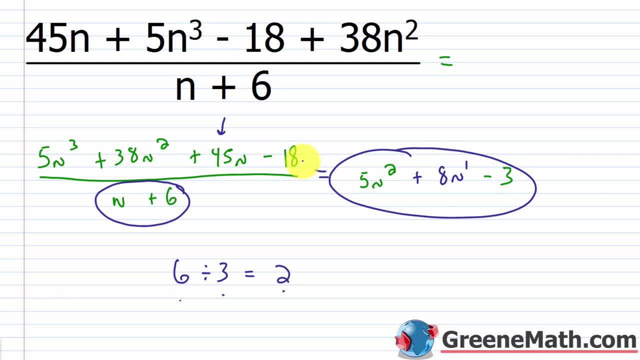 It's a more complicated equation, It's a more complicated example of that, but it's the same concept, All right, So let's go ahead and do this. If we had N plus six times five, N squared plus eight, N minus three. 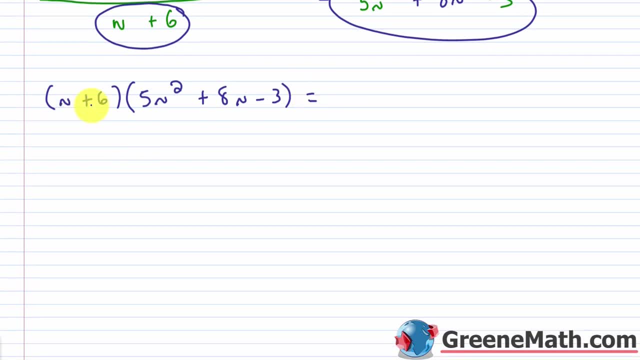 Scroll down a little bit. So N times five N squared is five N cubed. Then N times eight N would be plus eight N squared. Then N times negative three would be minus three. Then six times five N squared would be plus 30 N squared. 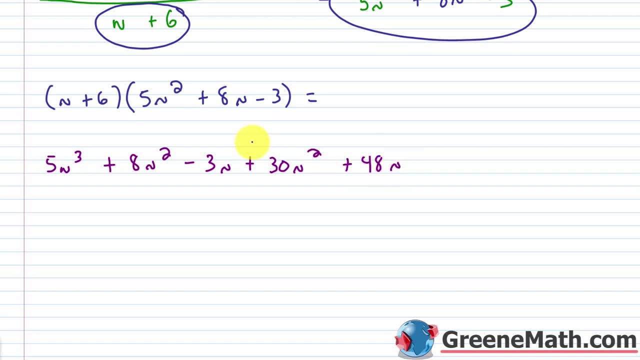 Then six times eight N would be plus 48 N, Then six times negative three would be minus 18.. All right, So if I combine like terms here, I'll have five N cubed And then eight N squared plus 30 N squared would be plus 38 N squared. 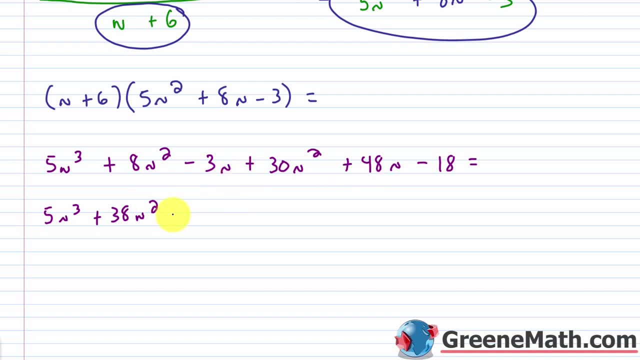 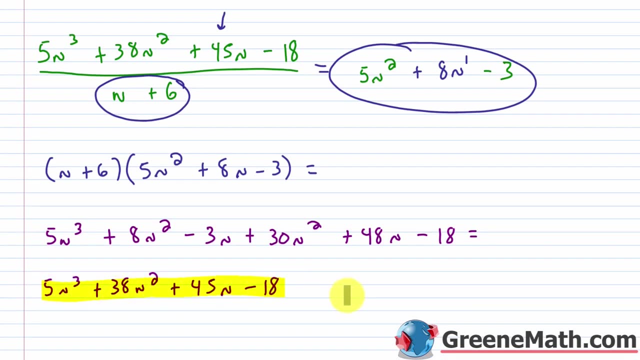 And then negative three N plus 48 N would be plus 45 N And then minus 18.. Now this is exactly what we had as our dividend: Five N cubed plus 38 N, squared plus 45 N minus 18.. So you can see that your division here is correct. 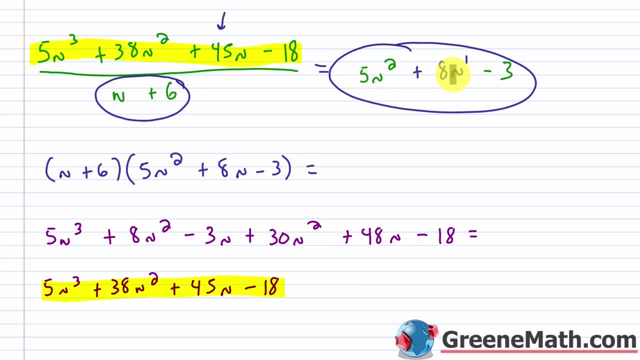 When I take the dividend and divide by the divisor, I get the quotient. So my quotient, which is here, times my divisor, which is here, gave me back my dividend, which is here, So you're always able to check your division. 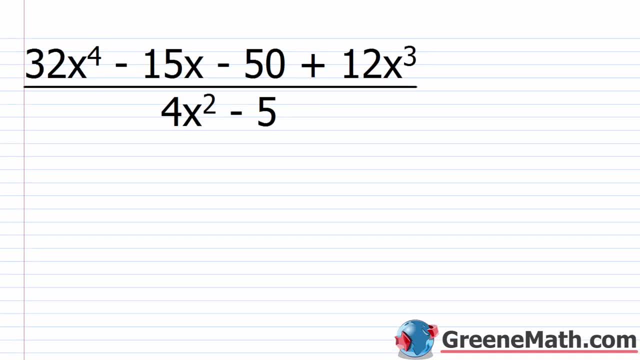 with multiplication. All right. Let's take a look at one where you have some division. Let's take a look at one where you have some missing terms involved. So we have 32 X to the fourth power, minus 15 X, minus 50, plus 12 X cubed. 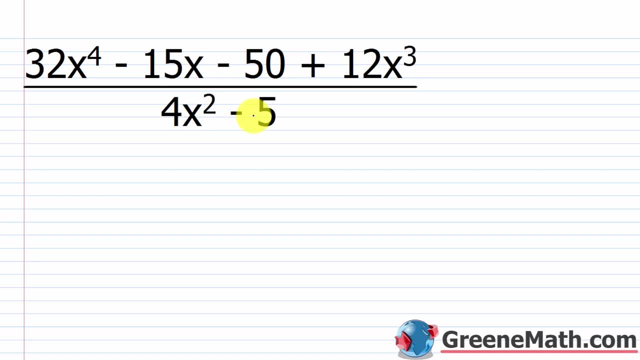 This is over four X squared minus five. So again, I want everything to be in standard form, And anytime I have some missing terms I want to put zero as a placeholder. So this is a perfect example of that. So in the numerator I've got 32 X to the fourth power. 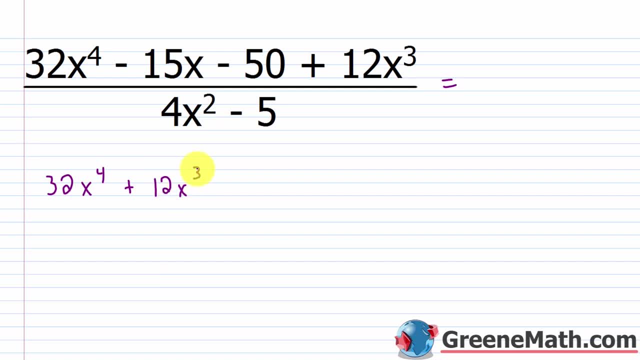 I've got plus 12 X cubed. Now, in order, I have X to the fourth X cubed. There is no X squared here, So I can't just leave it off. I've got to have it in there to do my division. 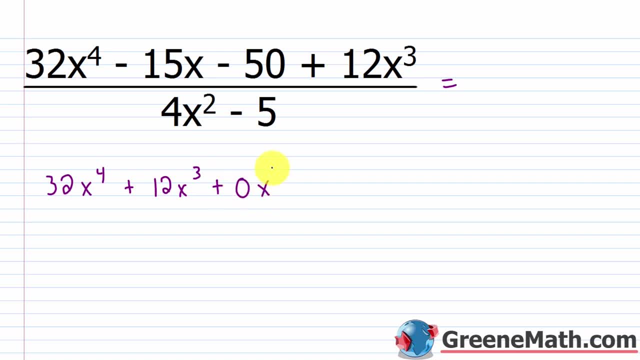 So what I want to do is I want to put plus zero X squared. It's just a placeholder, That's all it's doing, So we need to have that. Then I put minus 15 X and then minus 50.. So now this is in standard form and we. 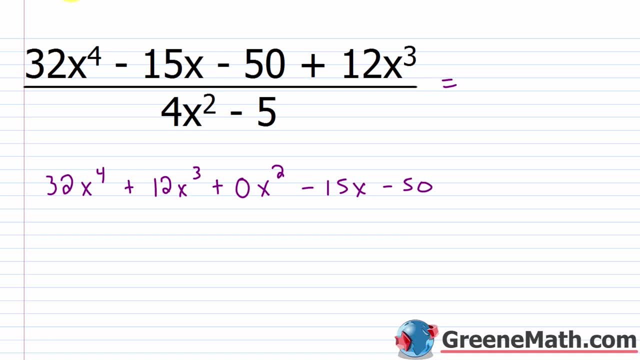 accounted for our missing term. All right, So for the divisor, here we have four X squared, minus five. Well, I have four X squared. I'm missing the X to the first power, So I'm going to put plus zero X and then minus five. 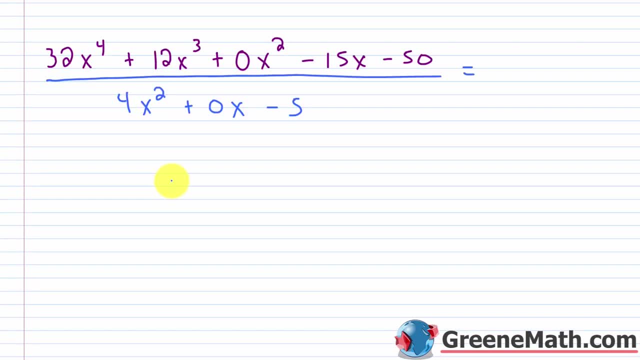 All right. So let's go ahead and set this up and we're going to do 32 X to the fourth power, plus 12 X cubed, plus zero X squared, minus 15 X minus 50.. I'm going to put that under our long division symbol. 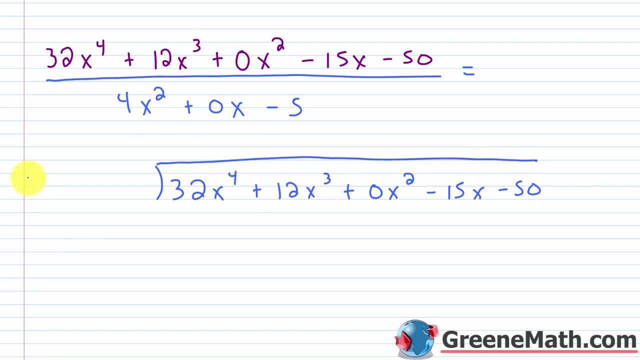 And then we're going to put our divisor out to the side. So four X squared plus zero, X minus five. So I'm going to go leading term into leading term. So what is? 32 X to the fourth, power over four X squared. 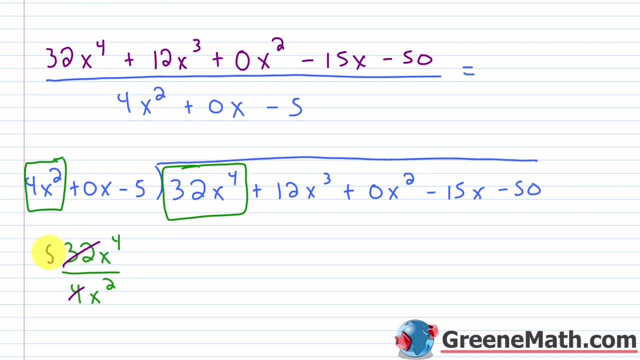 Well, I know that 32 divided by four would give me eight X to the fourth power. over X squared would be X squared. So I want to get eight X squared as an answer. Now, where am I going to put it? I'm going to put it over the X to the fourth power. 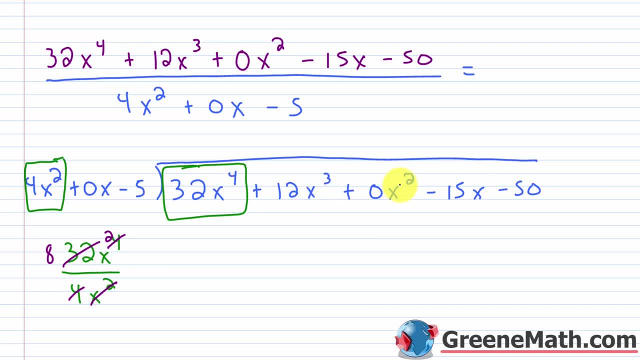 Not going to put it over the X cubed, Going to put it over the X squared. So I'm going to have eight X squared right there. Let me erase all this and we're going to multiply. Let me kind of scroll down so we have enough room. 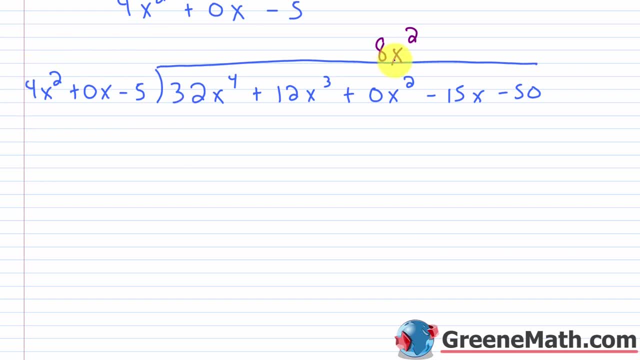 Remember, I'm going to multiply this by this whole thing. So eight X squared times four X squared Would give me 32 X to the fourth power. Eight X squared times zero, X would be plus zero X, cubed. And then eight X squared times negative five. 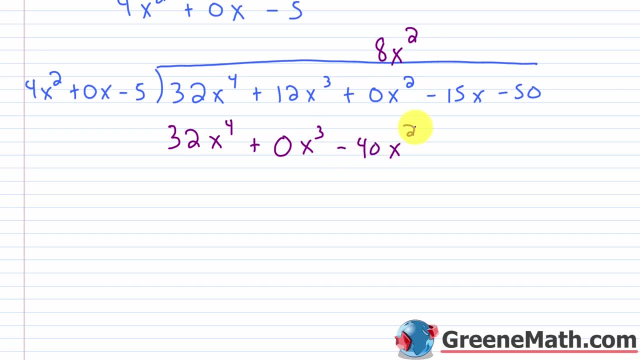 would be minus 40 X squared. Now I'm subtracting this whole thing away. So again I want to just change the sign of everything. So this would be minus, this would be minus and this would be plus. So let's put our little bar there. 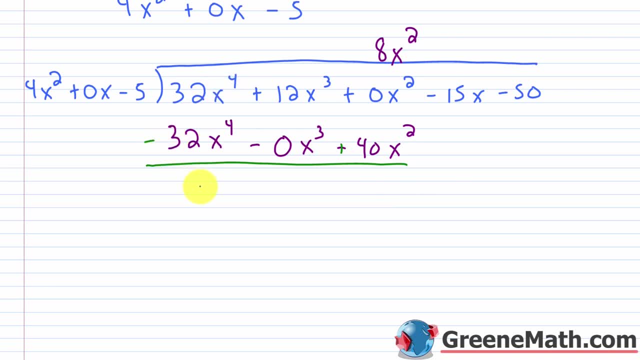 32 X to the fourth power. 32 X to the fourth power is zero: 12 X cubed minus zero X cubed is 12 X cubed. Zero X squared plus 40 X squared is 40 X squared. And then we want to bring down the next term. 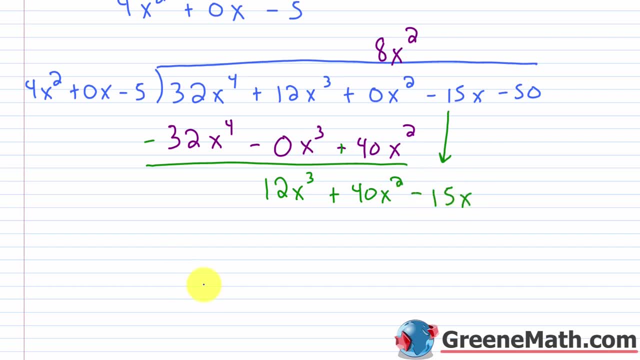 So bring down negative 15 X. Let's go ahead and go leading term into leading term. So what is 12 X cubed over four X squared? Well, we know that 12 divided by four X squared is 12 X cubed. 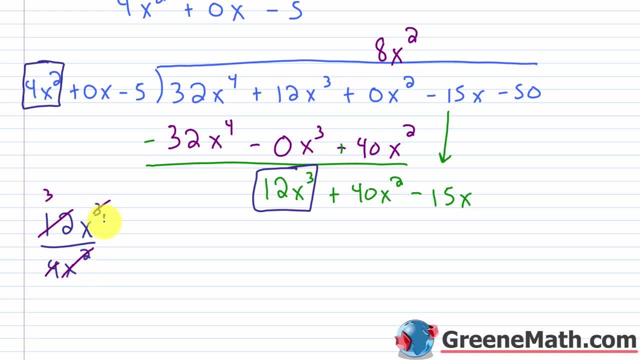 Four is three X cubed over X squared is X to the first power. So this would be three X to the first power or just three X. And again I want to do my multiplication. So if I do three X times four X squared. 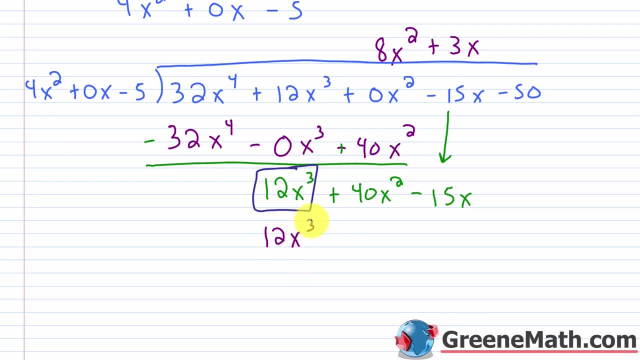 I'm going to get 12 X cubed. If I do three X times zero X, I'm going to get plus zero X squared. Then three X times negative five is going to give me minus 15 X. So we want to change the sign of everything and then add: 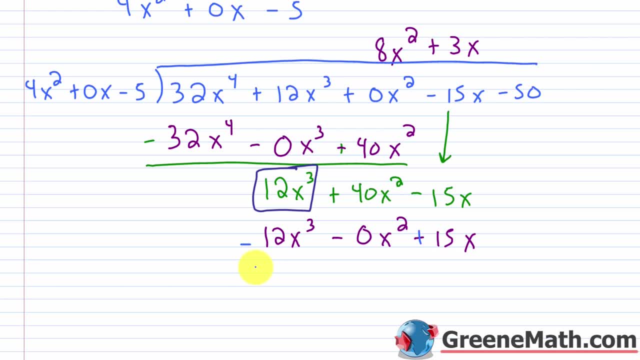 So this would be negative, This will be negative And this will be positive for our bar. So 12 X cubed minus 12 X cubed would give me zero. 40 X squared minus zero X squared would be 40 X squared. 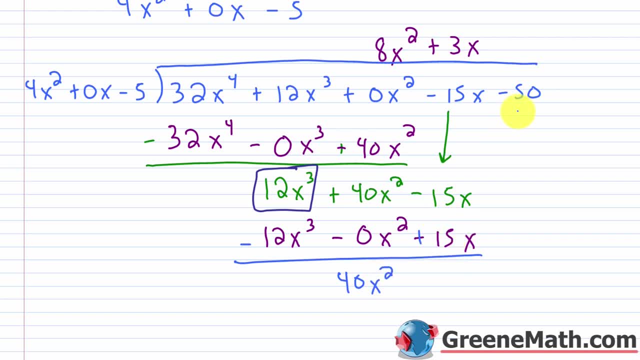 And then negative 15 X plus 15 X is zero. So I would bring down my next term here of negative 50.. And I would go leading term Into leading term, So I would have 40 X squared over four X squared. 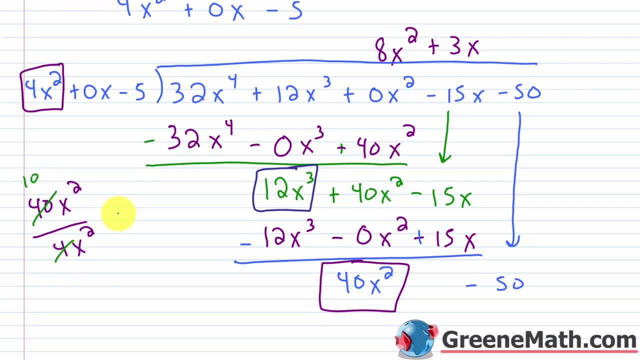 And so what's going to happen is this would cancel with this and I'll have 10 X squared over. X squared is one, So this would be plus 10.. Now I'd multiply. Let me erase all this. 10 multiplied by four X squared is 40 X squared. 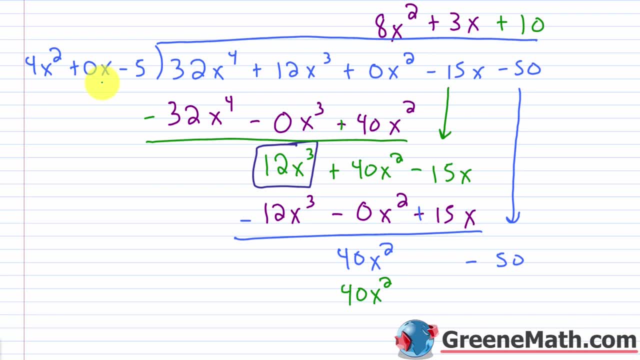 Then if I had 10 times zero X squared, remember zero X is just zero. So if I multiply 10 times zero, I get zero. So I could put a zero here, I could put a plus zero here and plus zero here. 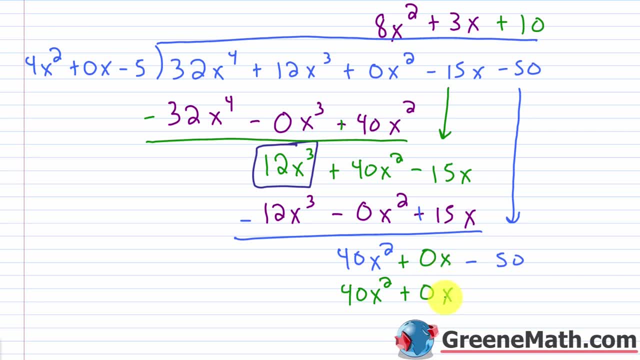 It doesn't matter, You can even put plus zero X and plus zero X just as placeholders, so things make sense. Then, lastly, I could do 10 times negative five, That's negative 50. And you can see that this is going to result in zero, right. 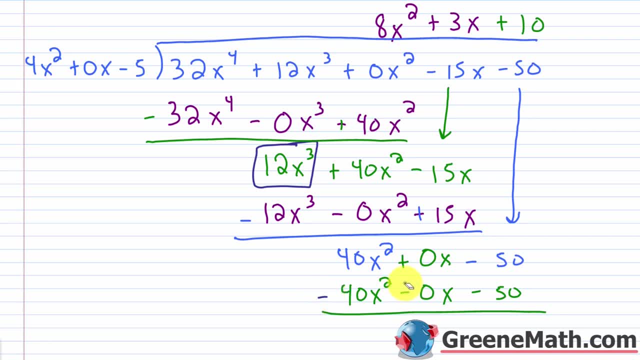 So, if I change the sign of everything, make this negative, this negative and this negative, Make this negative, this negative and this one negative and this positive. 40x squared minus 40x squared is 0.. 0x minus 0x is 0.. Negative: 50 plus. 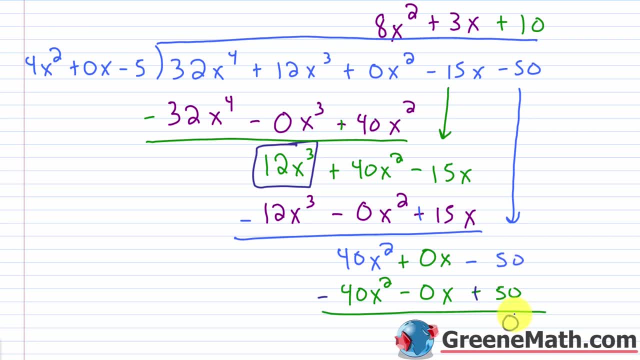 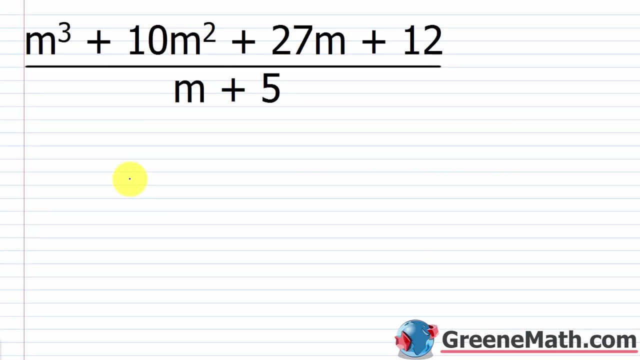 50 is 0.. So there's no remainder. here We end up with 8x squared plus 3x plus 10.. All right, let's just kind of wrap up the lesson now and just look at one with a remainder. So we have m cubed plus. 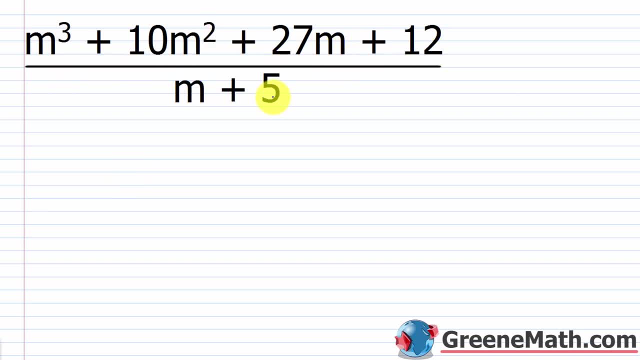 10m squared plus 27m plus 12 over m plus 5.. So everything's already in standard form for you and everything is there right. We're not missing any terms. So I can go straight into my long division here. I can just say: I have m cubed plus 10m squared plus 27m plus 12.. Okay, that's my. 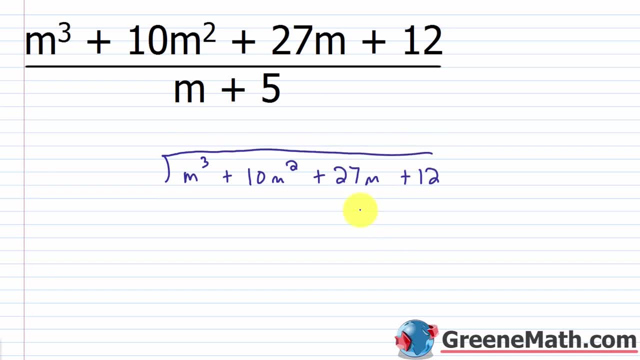 dividend, Putting that under my long division symbol and then out to the left, I'm going to have my m plus 5, my divisor. So I'm going to go leading term into leading term. So m goes into m. cubed how many times? 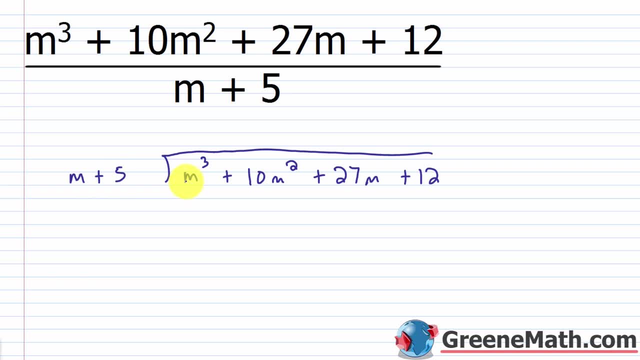 Well we know m cubed over m would be m squared. So that goes right here. We're going to have m squared m squared times. m is m cubed. m squared times 5 is plus 5m squared Again if I'm subtracting. 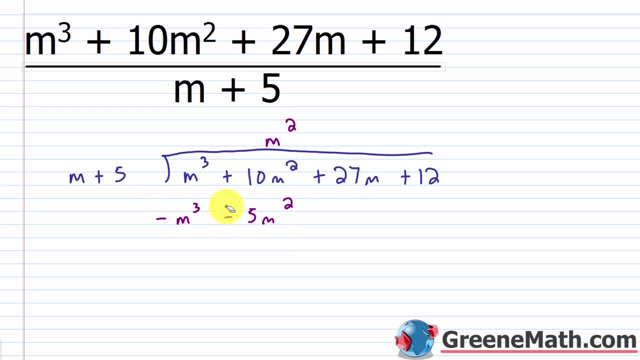 this whole thing away. change the sign of everything and then add m cubed minus m cubed is 0.. 10m squared minus 5m squared is going to give me 5m squared. The next thing I want to do is bring 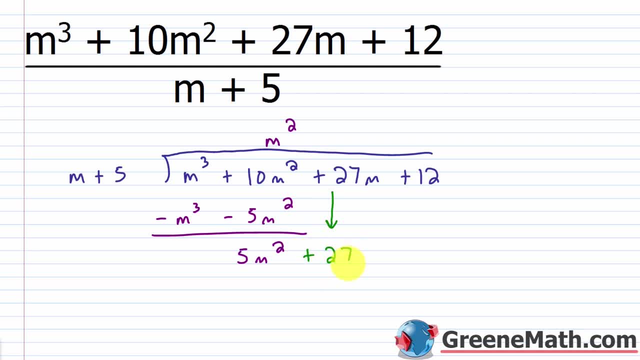 down this 27m, So plus 27m, And I just want to go leading term into leading term. So m goes into 5m, squared how many times? Well, we know m squared over m is m, So I would basically have that 5. 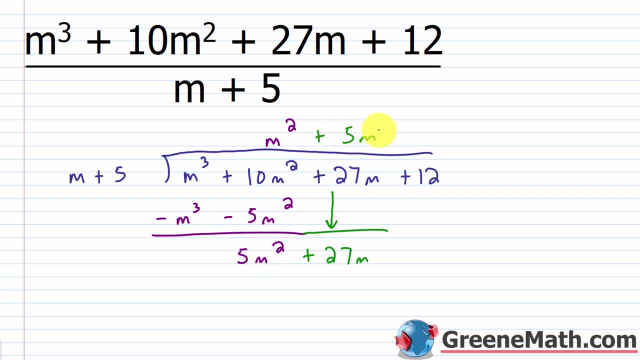 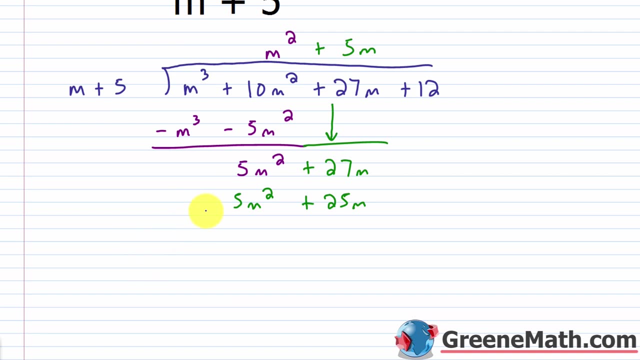 times m, So plus 5m. Then I multiply 5m times m, is 5m squared 5m times 5 would be plus 25m. Scroll down a little bit to get some room going. Now I want to subtract this away, So this becomes: 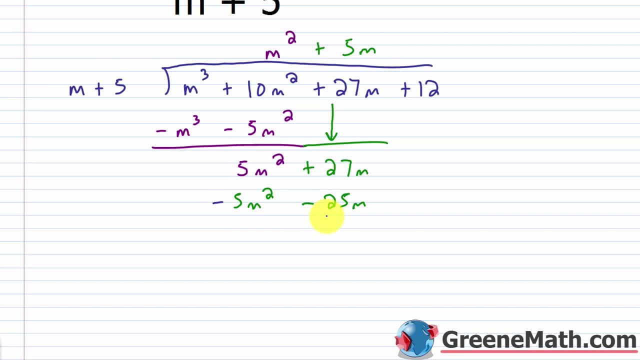 minus, This becomes minus. Change the sign of each term And then you can just add: So 5m squared minus 5m squared is 0.. 27m minus 25m is 2m. Bring down your last term there, So plus 12. And we're. 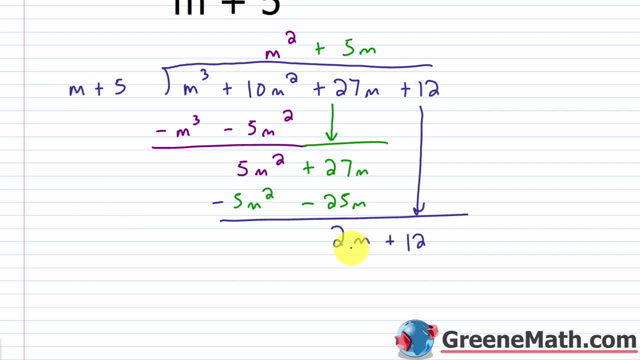 going to do one final time: leading term into leading term. So m into 2m. You think about 2m divided by m. The m's would cancel. You'd be left with 2.. So then 2 times m would be 2m, And then 2 times 5. 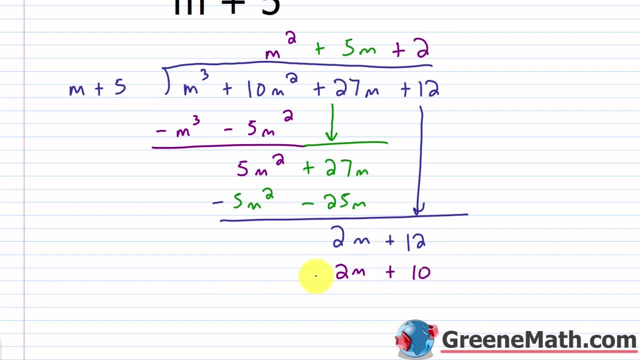 would be 10.. So we subtract this away. So this becomes minus, And this becomes minus And we can just add: 2m minus 2m is 0.. 12 minus 10 is 2.. Nothing else to bring down. This is a remainder. 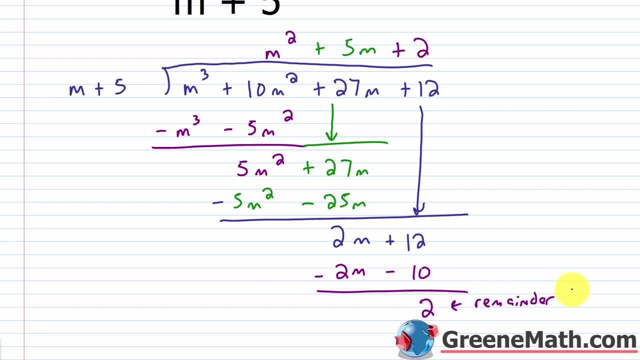 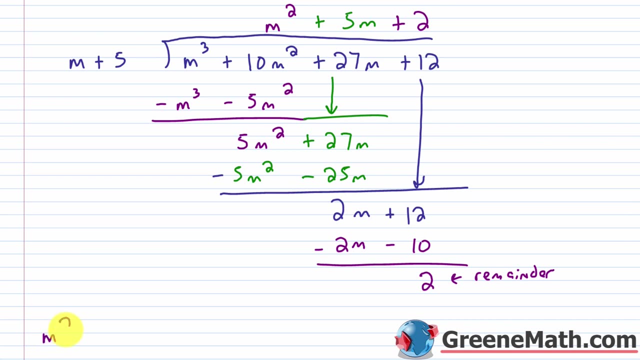 Remainder. Okay, We remember those from long division, Basic long division. Now all we need to do here is write it over the divisor. What that means is, if I write my answer, I have m squared plus 5m plus 2.. Then, plus, Here's my remainder: It's 2 over the divisor, which is m plus 5.. 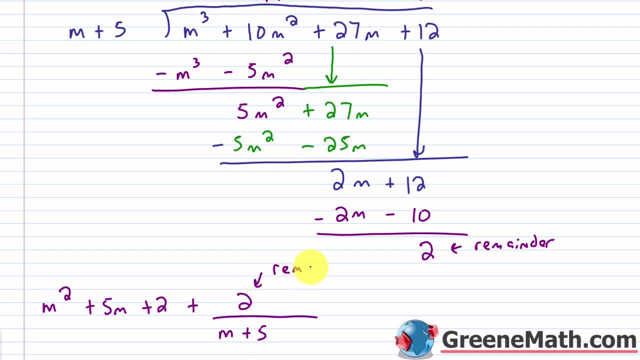 So this is the remainder And it's over the divisor. Okay, That's how you want to write this. Let's say you wanted to check the result. What would you do? Well, you could multiply this whole thing here by the divisor, Or you could multiply the quotient. 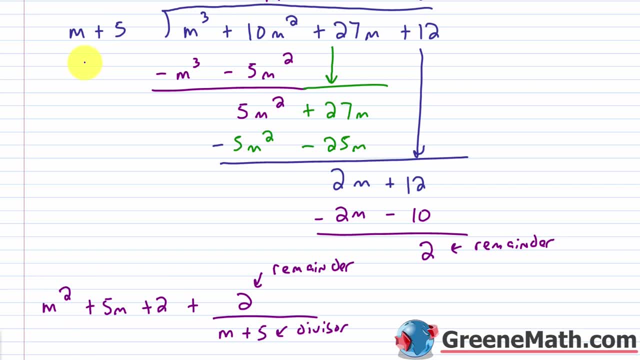 part by the divisor And then just add the remainder, So just say okay plus 2.. And it's the same thing. It's a little faster if you just multiply everything as it's presented here. So let me copy this. So let's say I just multiply this by the divisor. 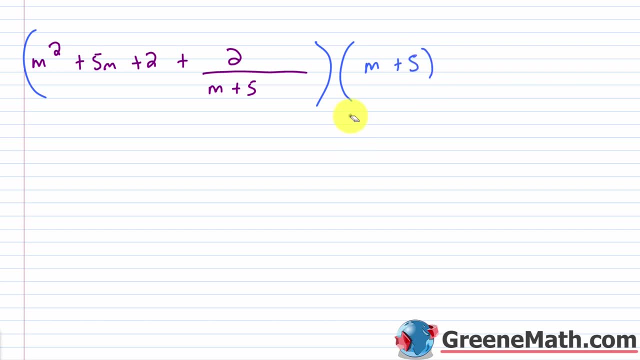 M plus 5.. So I could take and distribute this m plus 5 to each term, right? I could write this as: m squared times the quantity m plus 5.. Then plus 5m times the quantity m plus 5.. Then plus 2 times. 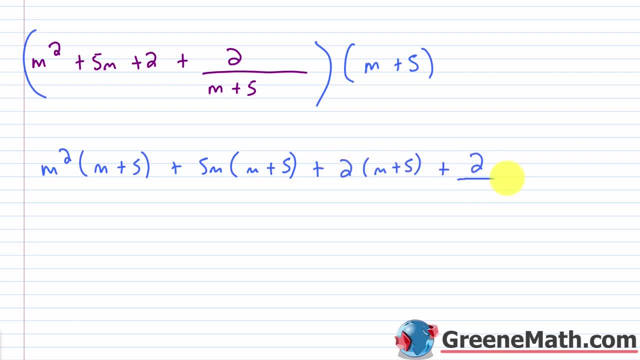 the quantity m plus 5.. Then plus 2 over m plus 5 times the quantity m plus 5.. Now the reason I do that is so that when we get down here this can be multiplied by the divisor. So I can take and: 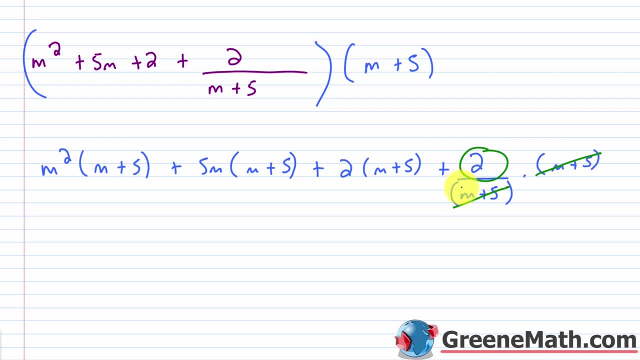 distribute this whole thing And then just add the remainder of the quotient part by the divisor. So that's why I'm saying it's the same either way. So that's why it's the same either way. If I just didn't have this in here and I did this multiplication and then I just added 2,. 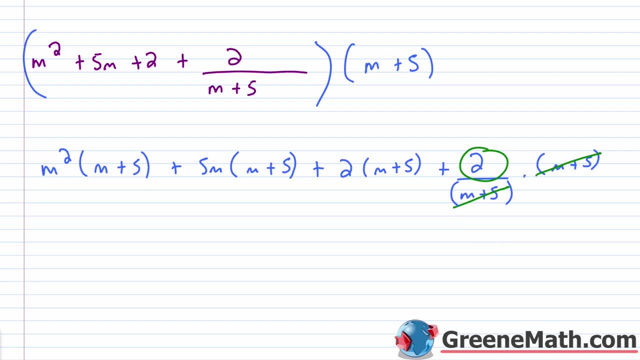 I'm getting the same thing, Okay, so that's why I'm saying it's the same either way. All right. so m squared times m is m cubed. plus m squared times 5 is 5m squared, Then plus 5m times m is 5m squared. Then plus 5m times 5 is 25m, Then plus 2 times m is 5m. 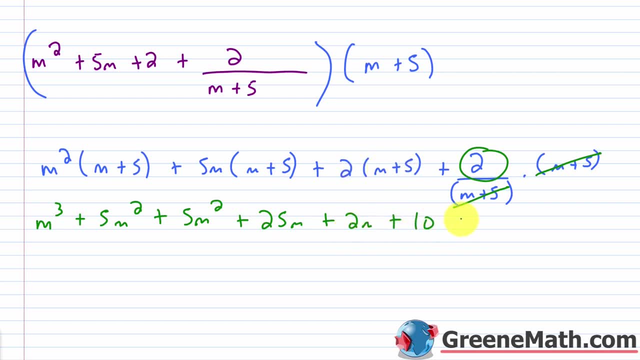 Then plus 2 times 5 is 10.. Then plus again, this cancels. I'm just adding 2.. So I'm going to end up with m cubed plus 5m squared plus 5m squared is 10m squared Plus 25m plus 2m is 27m Plus 10. 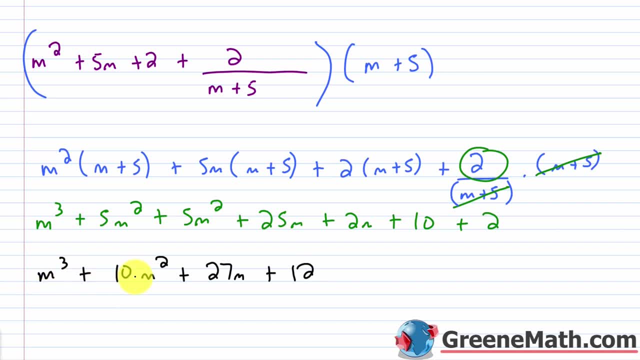 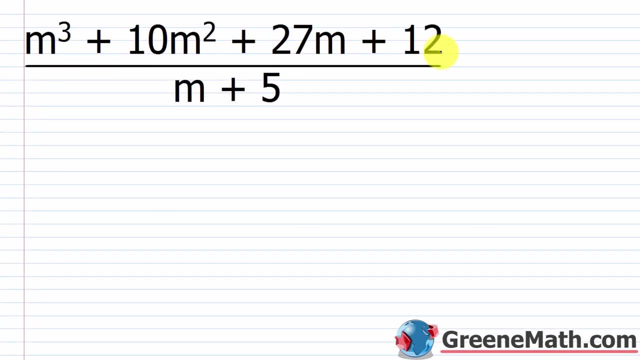 plus 2 is 12.. So I get m cubed plus 10m squared, plus 27m plus 12.. That's exactly what we had as our dividend when we begun: m cubed plus 10m squared, plus 27m plus 12.. 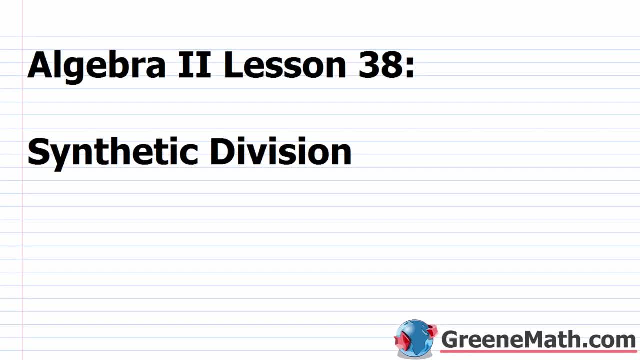 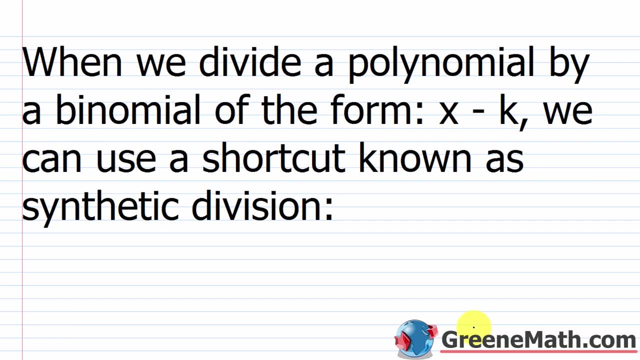 Hello and welcome to Algebra 2, Lesson 38. In this video we're going to learn about synthetic division. So for the majority of you who have only taken Algebra 1, and this is your first time around in Algebra 2,- you've probably never heard or seen anything about synthetic division. 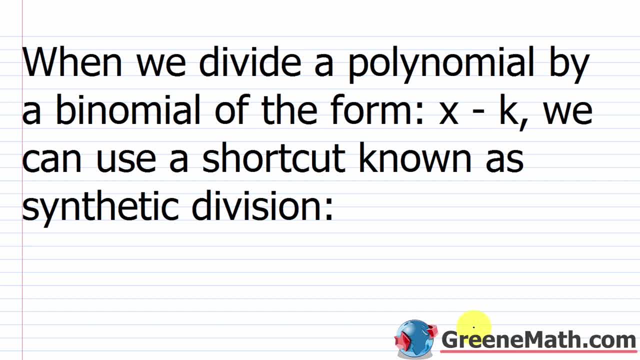 before. What I can tell you is it's just a shortcut for dividing polynomials in a certain scenario. So when we divide a polynomial by a binomial, we're going to divide it by a binomial, by a binomial. So when we divide a polynomial by a binomial, we're going to divide it by a binomial. 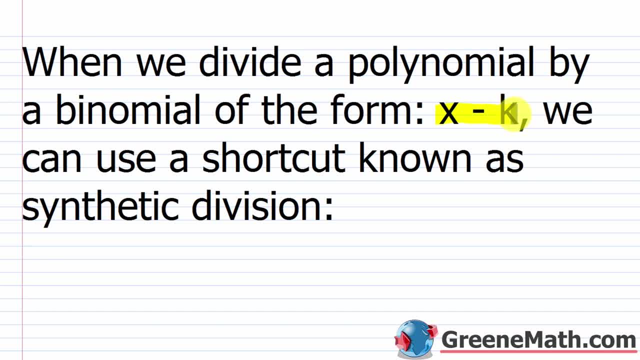 So when we divide a polynomial of the form- I'm going to highlight this- x minus k- we can use a shortcut known as synthetic division. This is a big time saver for us, so it's something you want to kind of memorize. So the procedure only works again if I'm dividing by a polynomial, that is, a. 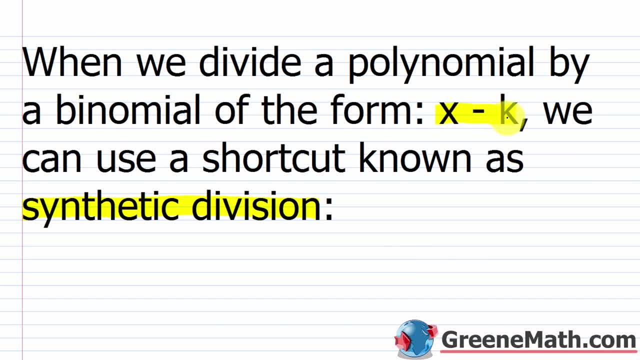 binomial of the form x minus k. So some examples: something like x minus 3,, something like x minus 12.. It could be x minus 2,. it could be x minus 3,. it could be x minus 2,. it could be x minus 2,. 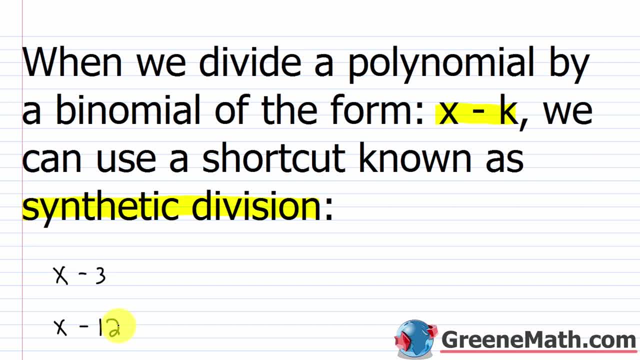 it could be x minus 2 billion, But it's got to be in that format. Now you might say: what if I have x plus something? That's okay too. If I had x plus 10, for example, I could rewrite this: 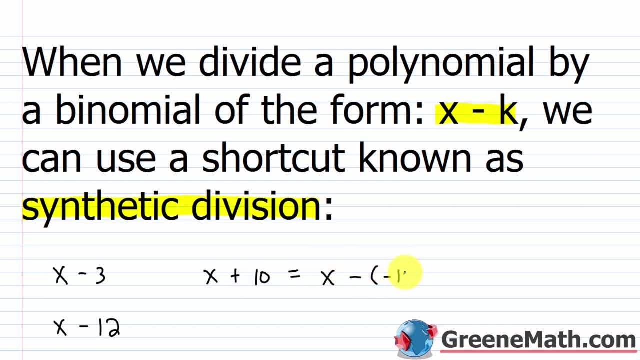 mathematically as x minus a negative 10. And you're going to see where we're going to do that when we get to our examples, What we can't have is an exponent on the variable that is not a 1. So, in other words, I can't say something like x squared plus 7, or something like x cubed. 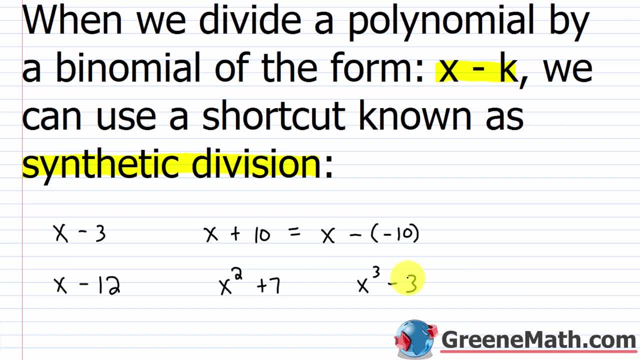 minus 3.. We also don't want to see a coefficient that is not 1 on the variable either. okay, So this is what we're looking for: Something in the format of x, or some variable could be y, z, q. 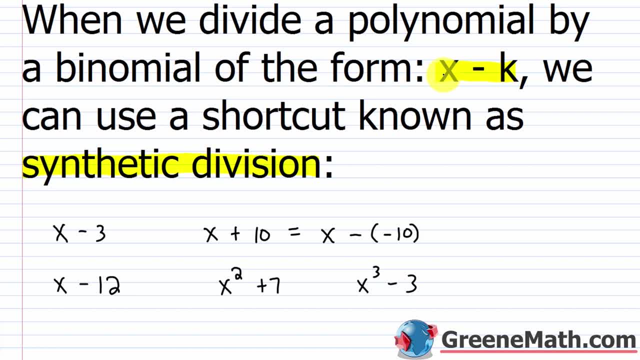 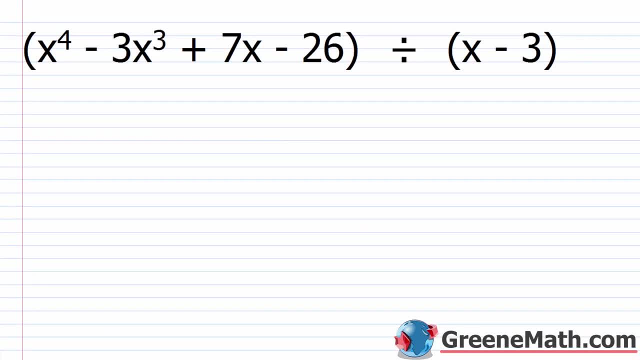 whatever you want to choose, minus some value- And again we could have plus some value by using this trick- minus a negative of that value. All right, so we all know how to divide x to the fourth power: minus 3x cubed, plus 7x minus 26.. 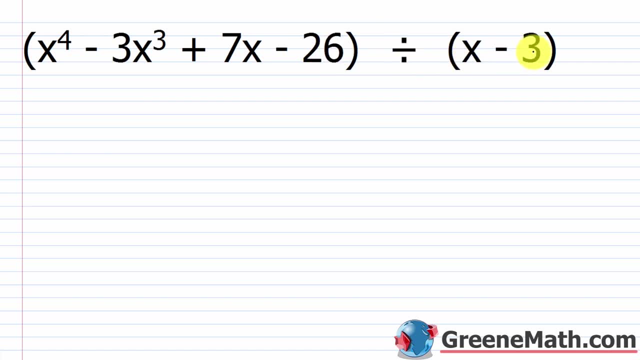 So what we're going to do is we're going to divide that by x minus 3 using long division. All right, we covered that in Algebra 1.. We just reviewed it in Algebra 2.. So you could pause the video now and you could do that and see what answer you get. then come back and see how we do. 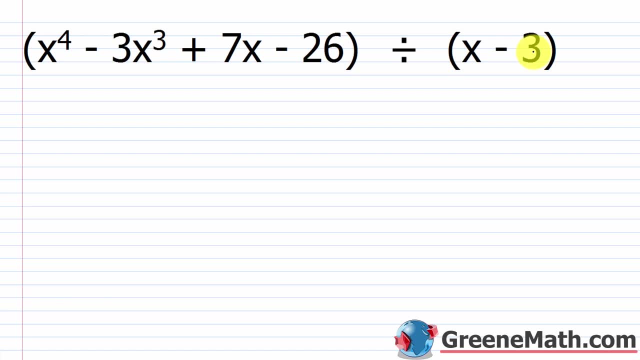 it with synthetic division, Or if you just want to follow along with the synthetic division, that's fine as well. The first thing you want to do- just like if I was doing polynomial long division- you want to make sure everything is in standard form And you want to make sure that, if you have 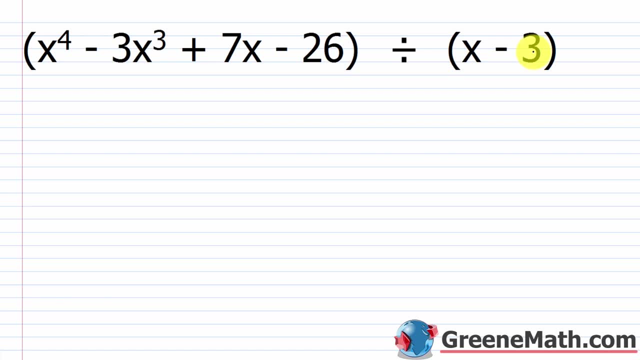 any missing powers for your variable. you want to make sure that everything is in standard form. So if you have any missing powers for your variable, that you put zero times that variable raised to that power. So, for example, here it's in standard form but I'm missing x squared. So I want to 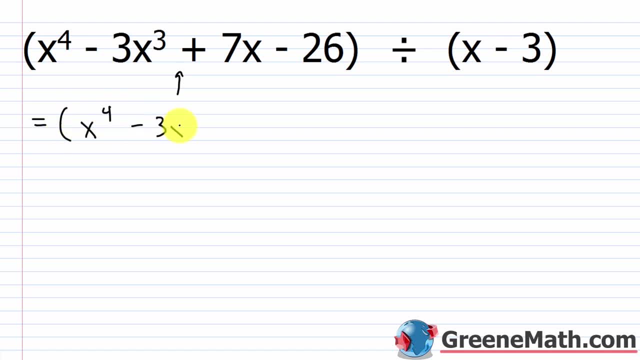 rewrite this and say: I have x to the fourth power minus 3x cubed, plus zero, x squared. Okay, zero is the coefficient for x squared, then plus 7x minus 26.. And this is divided by: we have x minus 3.. 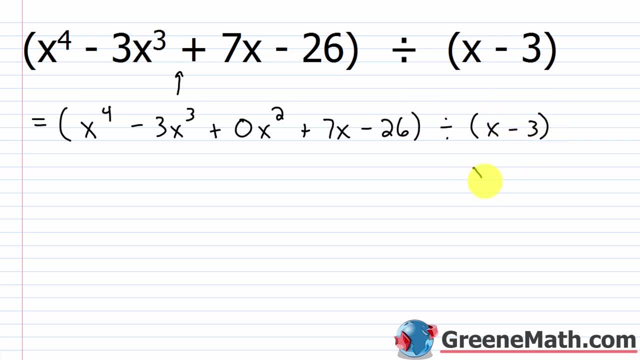 So this is in standard form And it's in the format of x minus k. In this case, three represents our value k. what we want to do now? we just want to do the numerical information from the dividend. I think about this kind of the. 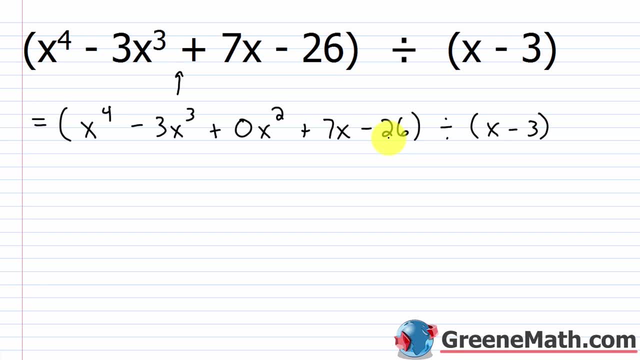 way that I think about matrices, When we solve a system of linear equations using matrices. we just took the numerical information out. we didn't really deal with the variables, So it's going to be the same thing. So let's set up a long division. 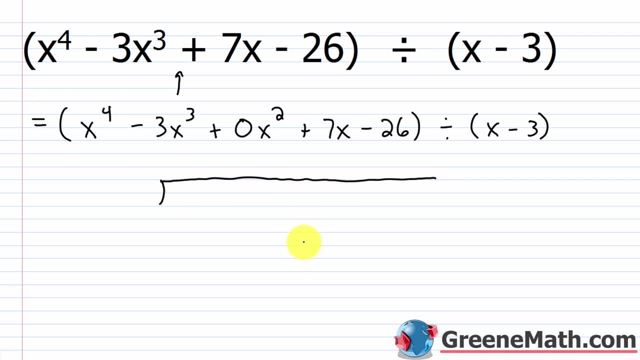 like we would. But instead of putting everything underneath, let's just take the numerical information. So what's the coefficient for x to the fourth power? Well, it's a one. So let's put that in. Then we'd have a negative three as the coefficient for x cubed, then we'd have a zero. 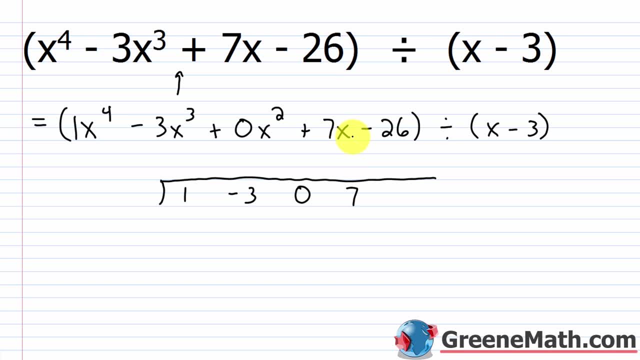 as the coefficient for x squared, then we'd have a seven as the coefficient for x to the first power. then our constant is negative 26.. So just the numerical information Now out here where we have a divisor. all we want to do again, if this is in the format of x minus k, we just want to plug. 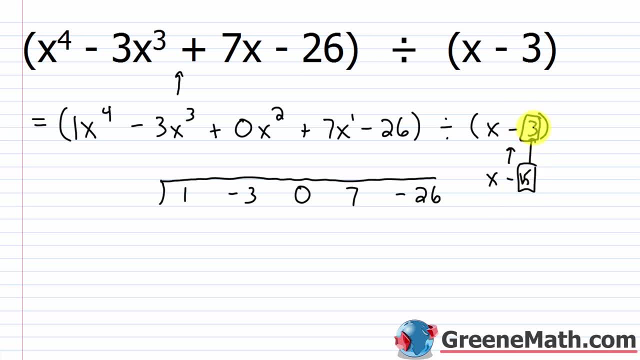 in whatever is in the place of k. All right, So in this case, that's the value three. Now here's where students get confused. If I have something that's already x minus some number, I just throw in this value. So this is going to be positive If I had, let's just say, for example, my divisor. 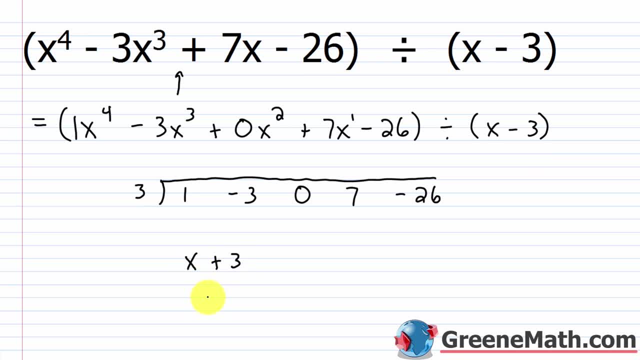 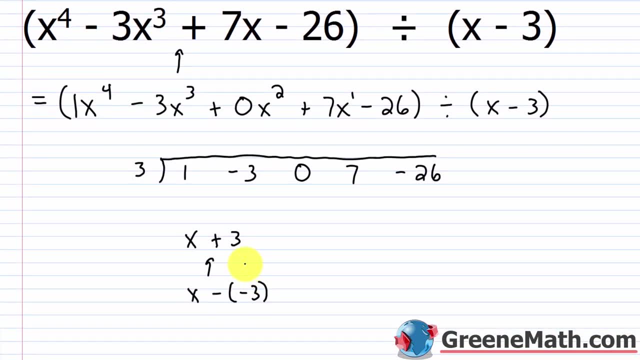 is x plus three. I just throw in this value, So this is going to be positive. If I had, let's just say, for example, my divisor is x plus three, So this is going to be positive. If I had, let's just say, for example, my divisor is x plus three, So this is going to be positive. If I had, let's just say, for example, my divisor is x plus three, So I just throw in this value, So we start out by rewriting that as x minus the negative of three. Okay, In this case, my value for k. if I line this up, x minus k is now negative three and that's what I use over here. That's a big source of confusion for students and that might not make sense for you right now, but again, as we work more examples, it's going to make sense. So right now, again, this is x minus three. It perfectly fits the format of x minus k. so we're going to get an x per square root of three. So what we're going to do is we're going to go over here and we're going to take a lot of these problems in the form of the equations to 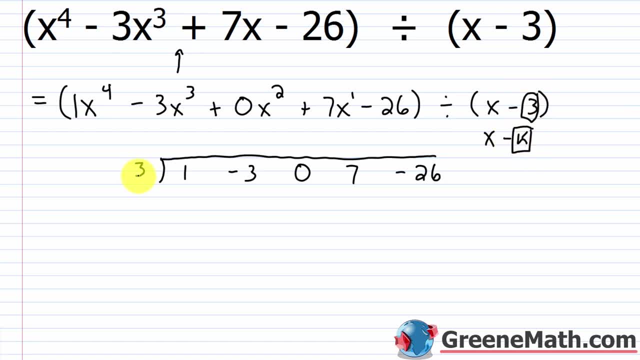 So I just plug in this three right here. Okay, that's all I'm looking to do Now. the other thing I wanna tell you is there's many ways to write this In your textbook or in your class or in your tutoring session. 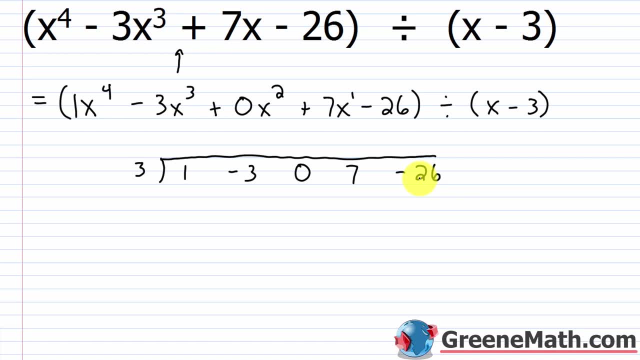 or wherever you get this information. you might see this drawn differently. It's the same procedure either way. Do it however you want to. It's just a matter of just getting the right answer. okay, Now, once you've set this up, 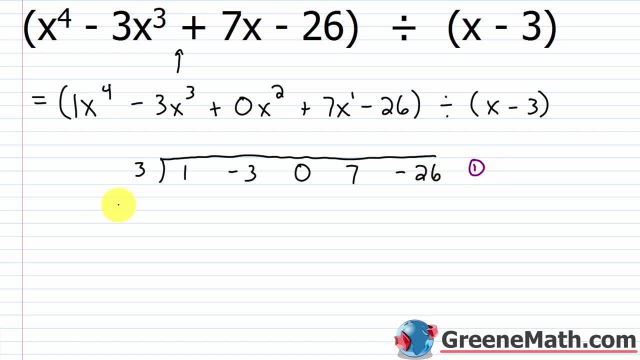 there's gonna be three rows involved, So this is kind of row one. You're gonna need to leave a little space for row two. Then you draw a little line down here and this is going to be row three below it. okay, So you've got row one, row two, row three. 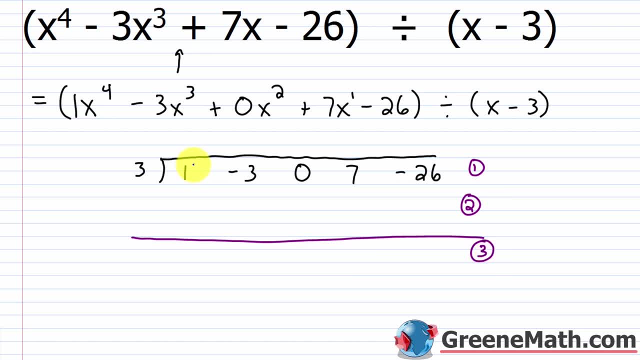 Now the very first thing you're gonna do is take your leftmost number that's under this long division symbol, and you're gonna drop it all the way down to row three. So this is a one coming all the way down. Now the procedure is very simple. 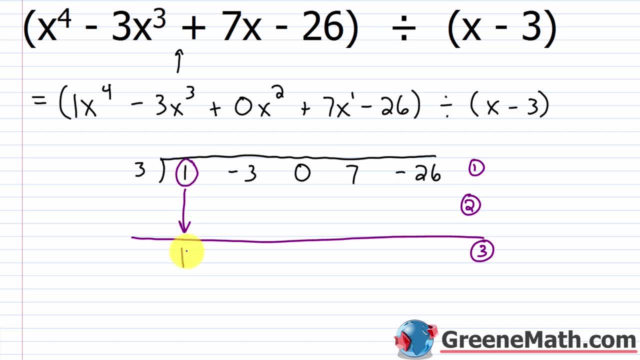 It kind of repeats itself over and over again. Once I've dropped this down, I'm just gonna multiply Three times one is going to give me three, So I'm gonna write it in the next position here, So in this next column in row two. okay, 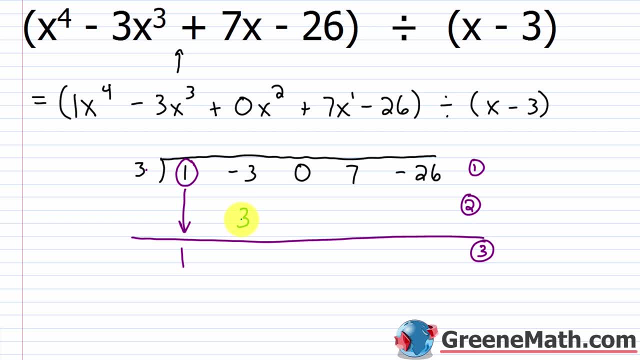 So now I have negative three and three there. All I'm gonna do is I'm just gonna add: So negative three plus three is zero. Now I'm gonna multiply again: Three times zero is zero. Put the result here. I'm just going one column to the right. 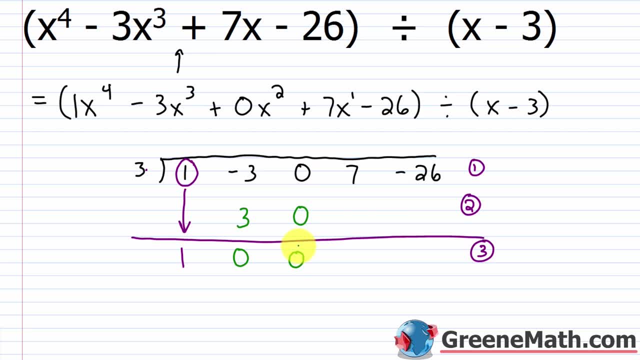 and I'm doing the same thing. So now I'm gonna add: Zero plus zero is zero. You guessed it. Now I'm gonna multiply Three times. zero is zero. Put that right here, one column to the right, and add: Seven plus zero is seven and I'm gonna multiply. 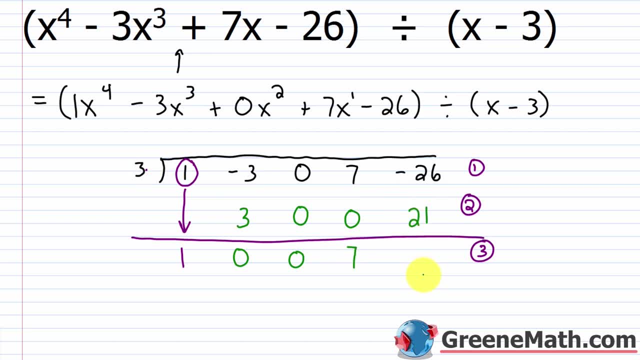 Three times seven is 21.. Put that right here. one column to the right. then add Negative 26 plus 21 is negative five. So you see how quickly we went through this and I can tell you we already have our answer, okay. 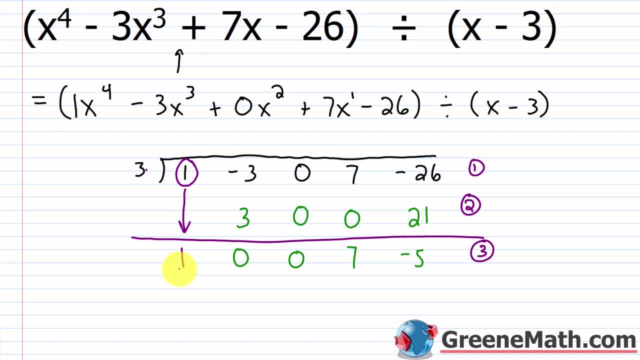 You don't see that yet, but we already have our answer. These are the coefficients and the remainder. So if I start all the way to the right, this is going to represent my remainder. Then if I move to the left, this represents my constant. 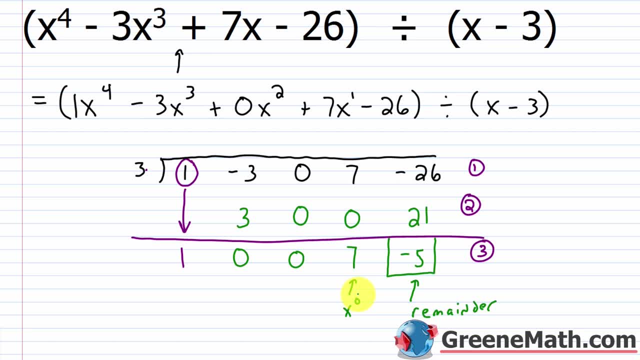 or my coefficient for x to the power of zero. As I go to the left, the exponent on x is gonna increase by one. So this is the coefficient for x to the first power. This is the coefficient for x squared and this is the coefficient for x cubed. 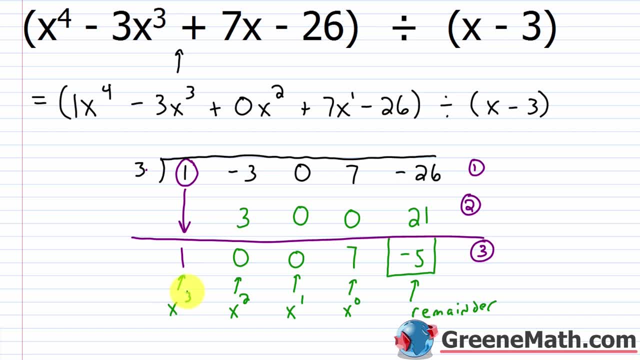 Now I can also start from the left and go to the right. Again, everything's in standard form, so we know that this would be the highest exponent and it would decrease by one as I move to the right. So I could have figured out the same thing. 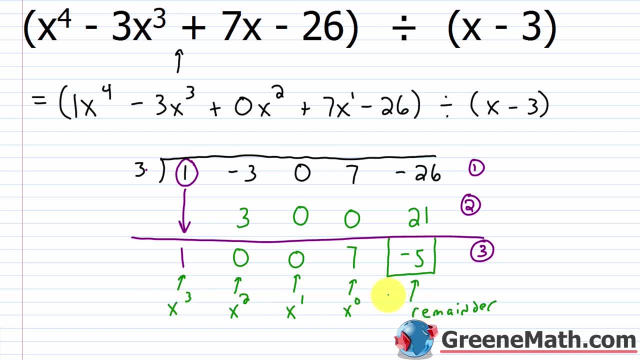 just by knowing that when we get our results it's gonna be one degree less than the dividend. Now, in the dividend the highest exponent was a four, So the degree was a four. Here the highest exponent is going to be one less. 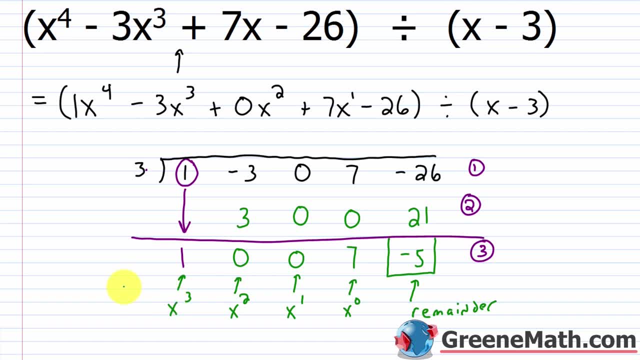 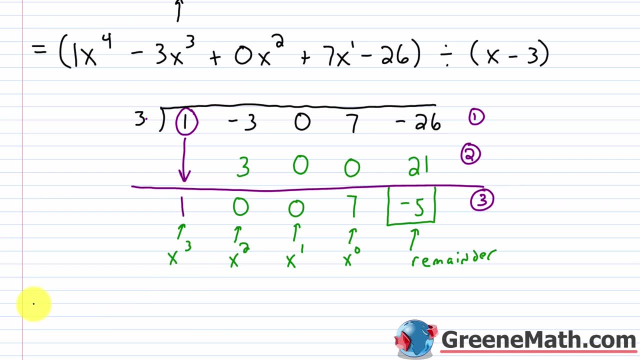 so a three. So I would begin with x cubed. Now I have the numerical information so I could just write my answer. So what I would do is I would say: okay, I have one as the coefficient for x cubed. 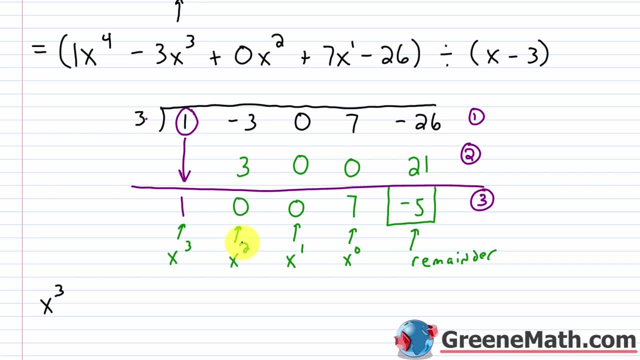 So that would be one x cubed or just x cubed. I have zero as the coefficient for x squared. Zero x squared is just zero, so I don't need to put that. I have zero as the coefficient for x to the first power. 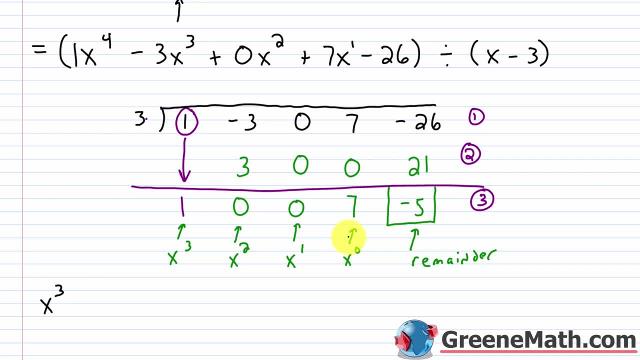 Zero times x is just zero. I don't need to put that. I have seven as the coefficient for x to the power of zero. X to the power of zero is just one. It's like seven times one is just seven. Seven is my constant. 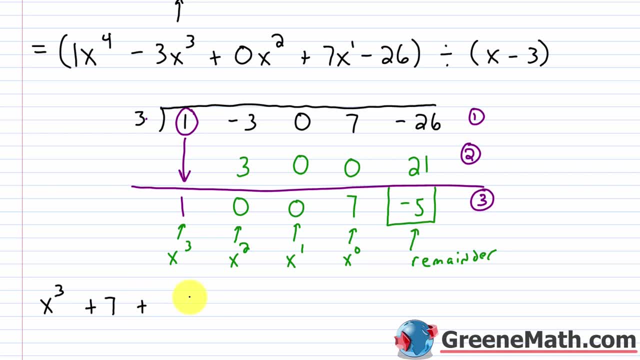 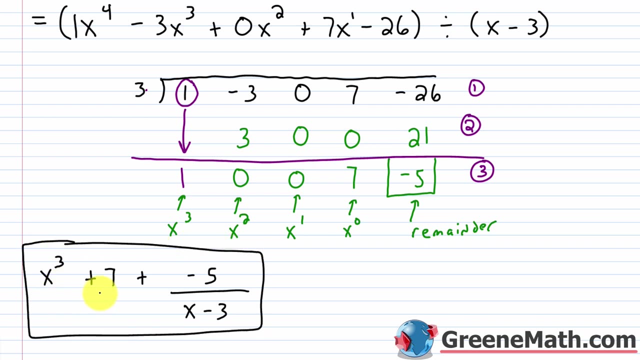 I have one x cubed plus seven And then I have my remainder, So plus you have negative five and you place this over your divisor, which is x minus three. So this is your answer, right here: It's x cubed plus seven plus negative five over the divisor x minus three. 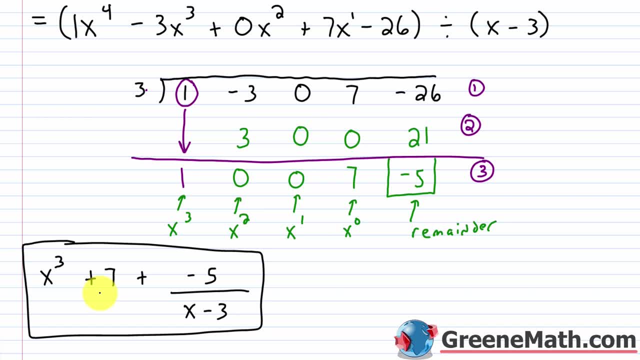 And you can see how much quicker that would be versus setting up a long division and going through and having to involve the variables. Just working with the numbers is definitely quicker. All right, Let's go ahead and take a look at another one. I know some of you will kind of be like: well, I'm a little fuzzy on that. 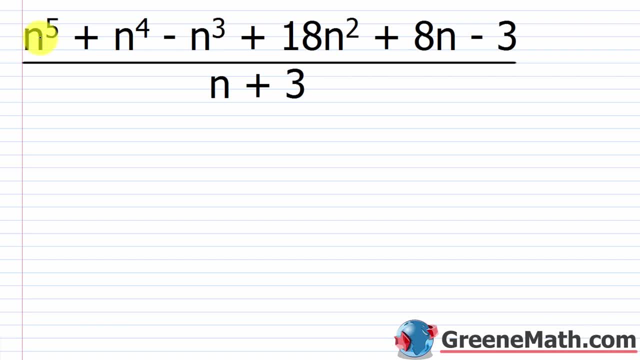 It just takes practice. So we're going to work a lot of problems here. So we have n to the fifth power plus n to the fourth power minus n. cubed plus 18n squared plus 8n minus three, This is over n plus three. 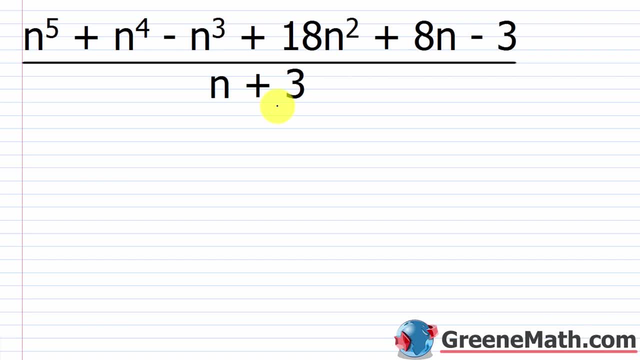 So again, I'm looking for standard form and I'm looking for no missing powers on the variable n. So I have the fifth power, fourth, third squared and first power. I'm going to go ahead and do that, All right. 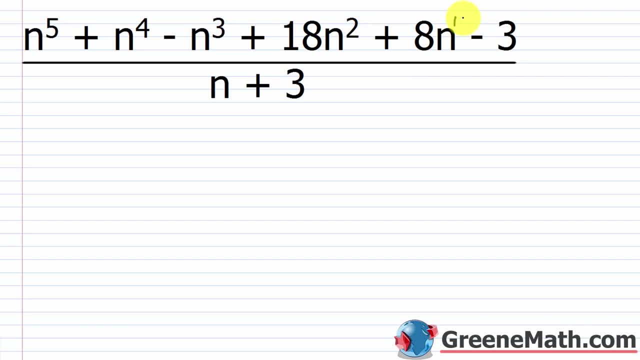 So I have the fifth power, So I'm good there. And everything is in standard form, so I'm good there. So now I'm just going to set up my synthetic division. So underneath this long division symbol, I'm going to put all the numerical information. 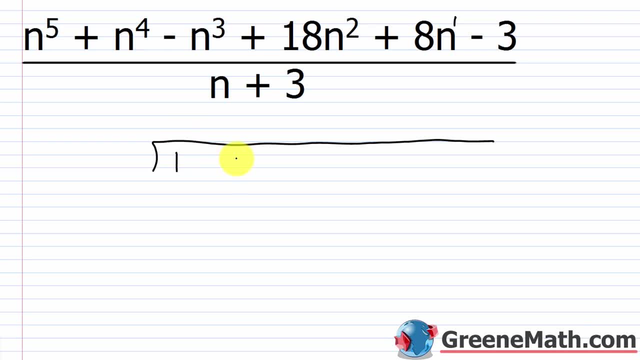 So the coefficient for n to the fifth power is one, Then the coefficient for n to the fourth power is one. The coefficient for n cubed would be negative one. So let's put a negative one there. Then the coefficient for n squared is 18.. 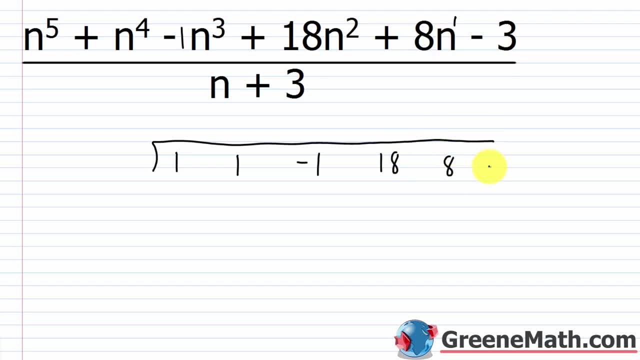 Then the coefficient for n to the first power is one, Then the coefficient for n to the first power is eight, Then my constant is a negative three. So out here, what am I going to put? Again? this is where students make a mistake. 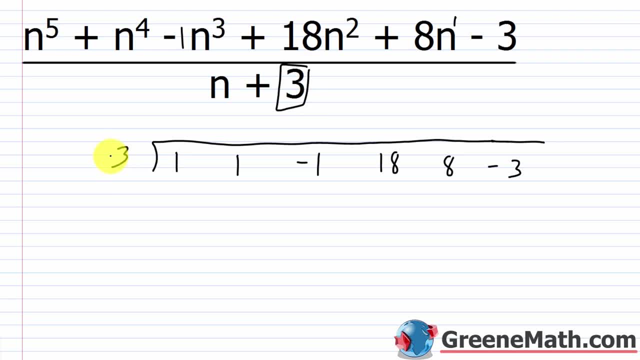 They go: okay, I'm just going to throw a three over there. That's wrong. We want in the format of x minus k and we want k to go right there. Now, in this case I have. let's just say, for example, this isn't n. 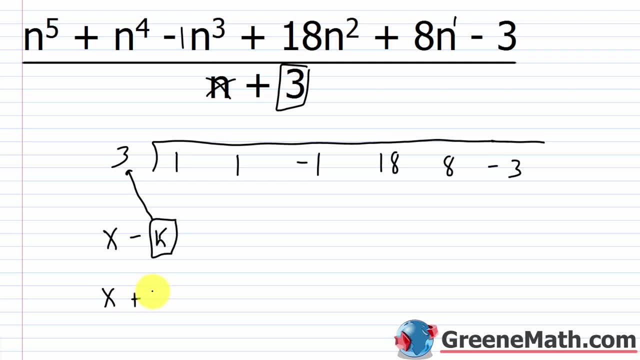 Let's just say this was x. Okay, If I have x plus three, I need to rewrite it to match this format: x minus a negative three. This right here is representing k, and so k has to be negative three in this scenario. 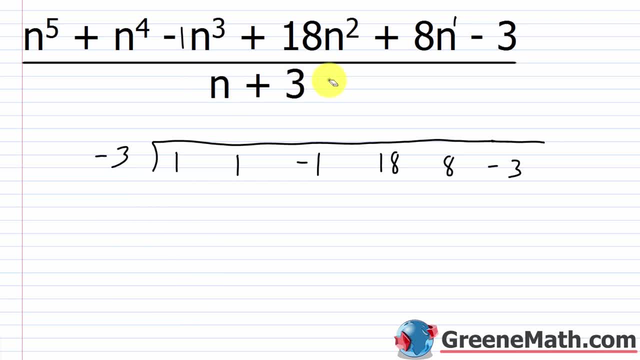 Take the time to understand that, because that's a common source of confusion and it leads to a lot of wrong answers. This number right here has to be based on what is given to you there. If you have some variable plus a positive number, this is going to be the negative of. 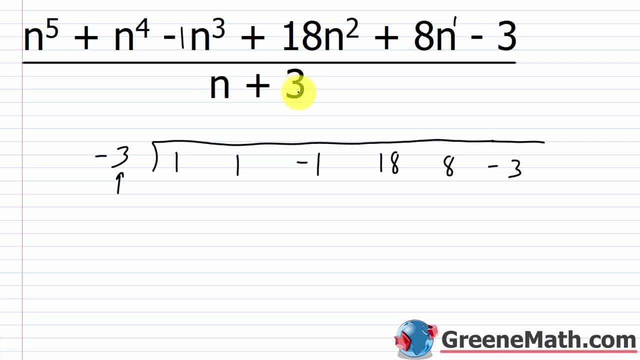 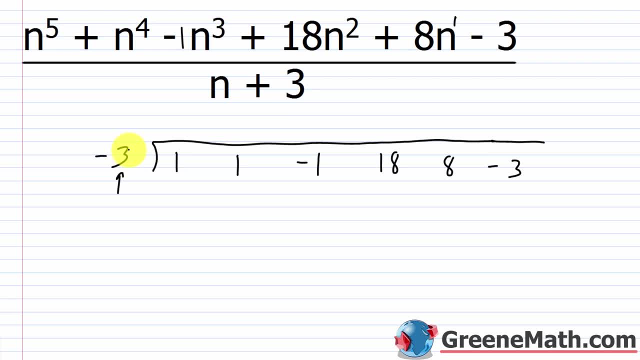 This is going to be just the number. okay, that's being subtracted away. Alright, so once we have that again, we have three rows going on, so let's kind of make a little bar here and let's drop this guy into row three to begin. 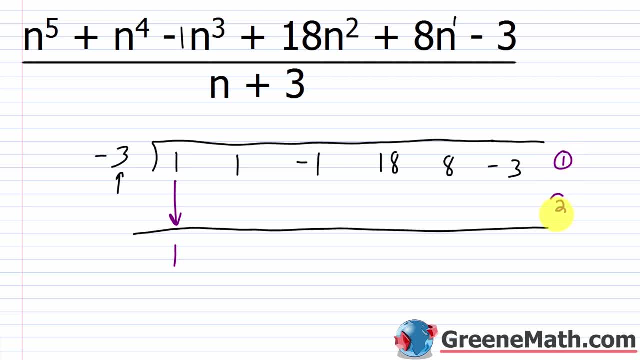 And I can number the rows. you don't have to. It's not traditional to, But I just do it so that you understand what I'm saying. So I'm dropping this first one all the way to the left into row three. That's the first thing you do. 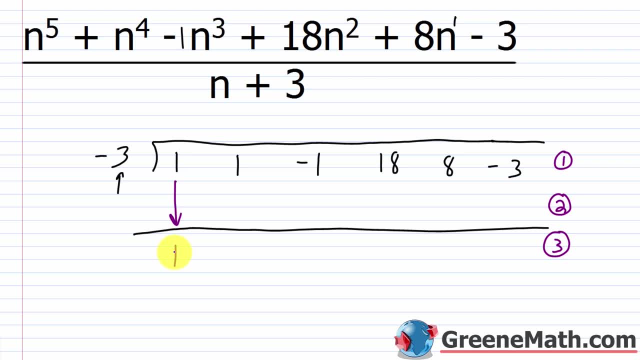 And then you start a series of multiplication and addition. So I multiply negative 3 times 1 to kind of get the ball rolling. That's going to give me negative 3.. Now I'm going to add 1 plus negative 3 is negative 2.. 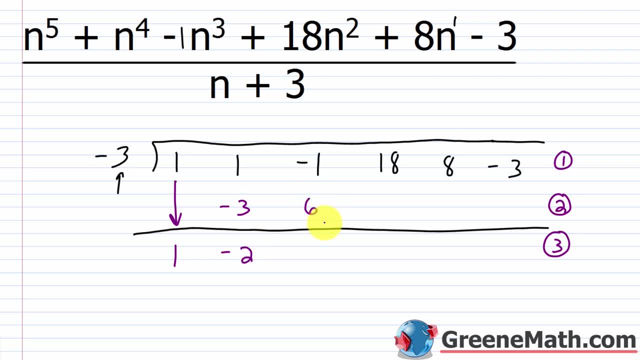 Now I'm going to multiply Negative 3 times negative: 2 is 6.. Now I'm going to add Negative 1 plus 6 is going to be 5.. Now I multiply Negative 3 times 5 is negative 15.. 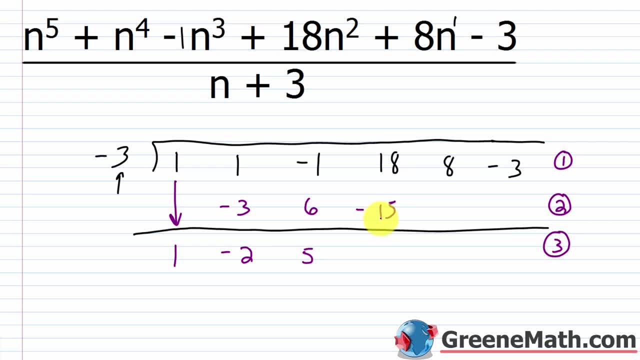 Now I add 18 plus negative 15, or 18 minus 15, is going to be 3.. Now I multiply Negative 3 times 3 is negative 9.. Now I add 8 plus negative, 9 is negative 1.. 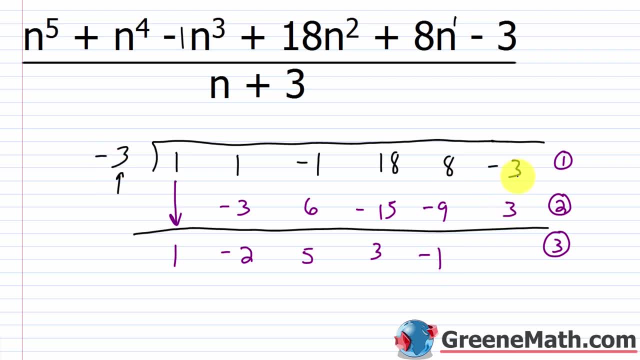 Now I multiply Negative 3 times negative, 1 is 3. And then negative 3 plus 3 is 0. Since we have a 0 in the final position, that means we have no remainder. Okay, no remainder. We know already that this will be 1 degree less than the dividend. 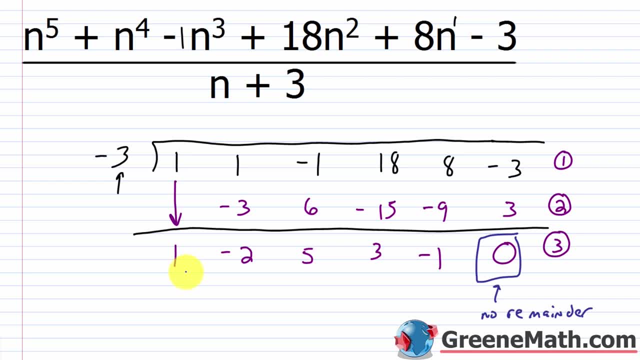 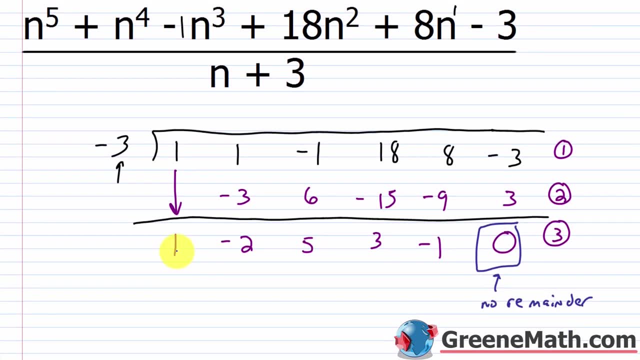 The dividend has a degree of 5.. This will have a degree of 4.. So that means the highest exponent would be a 4.. So 1 is the coefficient for n to the 4th power. So if this is the coefficient for n to the 4th power, we just have n to the 4th power. 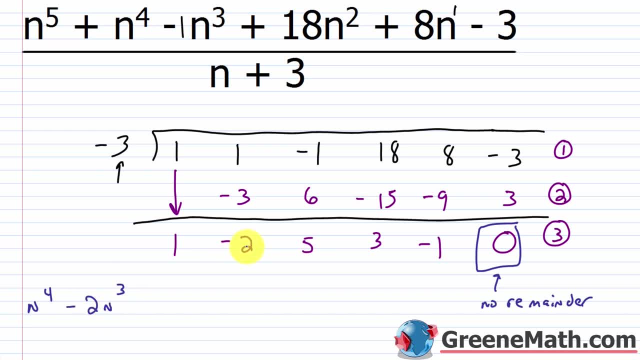 Then I would have minus 2n cubed, Right, This is the coefficient for the n cubed. This is the coefficient for n squared. So then plus 5n squared, And then this is the coefficient for just n to the 4th power. 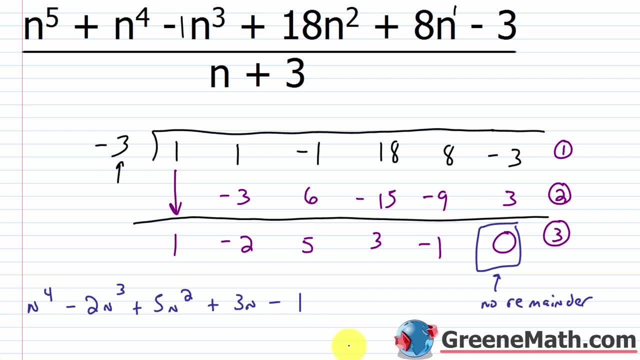 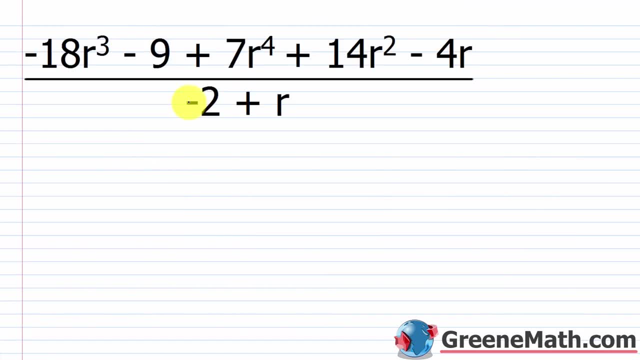 So plus 3n, And then that's my constant, So minus 1.. Again, that's 0 there, So there's no remainder. So this would be your n And that would be the answer for the problem. All right, for the next one we're looking at negative 18r cubed minus 9 plus 7r to the 4th power plus 14r squared minus 4r. 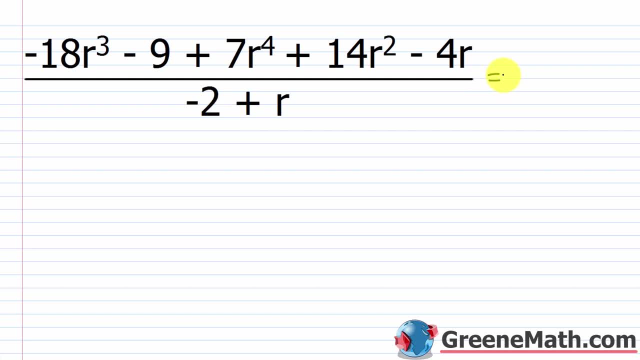 This is over negative 2 plus r. So the first thing I want to do is write each one of these, the numerator and denominator, in standard form. So I'll have 7r to the 4th power, to begin Right. 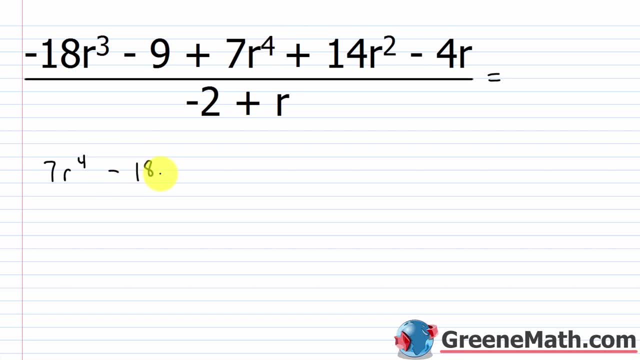 4 is the largest exponent, Then next I'll have minus 18r cubed, Then I'll have plus 14r squared, Then after that I'll have negative 4r, Then lastly I'll have minus 9.. 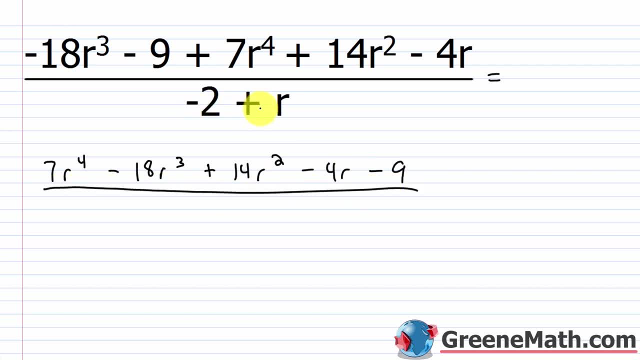 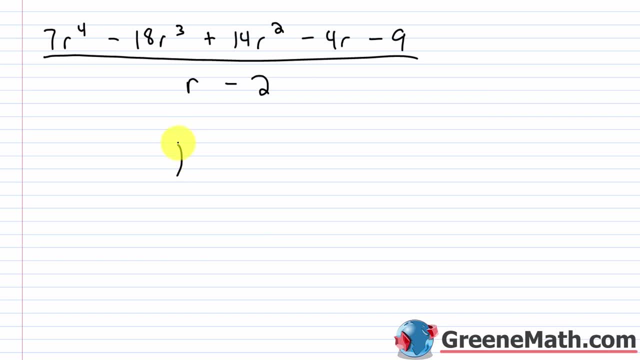 Okay, then this is over. We have negative 2 plus r. We need to switch that. We need to write this as r minus 2.. So now this is in standard form And I'm going to set up my little long division symbol here. 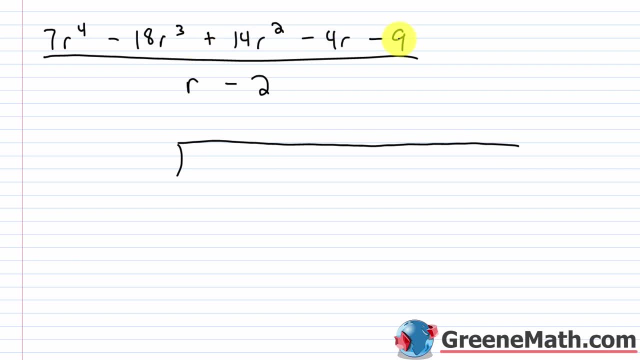 And I'm going to take the numerical information out of the numerator or the dividend. So I want a 7.. I want a negative 18.. I want a 14.. I want a negative 4. And I want a negative 9.. 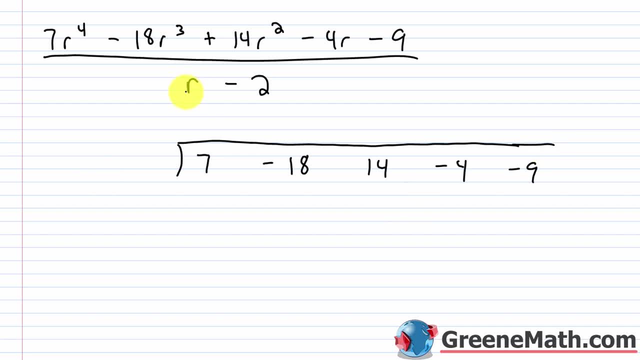 Then over here. remember this follows the format of a variable minus a positive value. We just take this value right: x minus k, k gets plugged in right there. So we just want a 2 right there. And one more time. I just want to cover this. 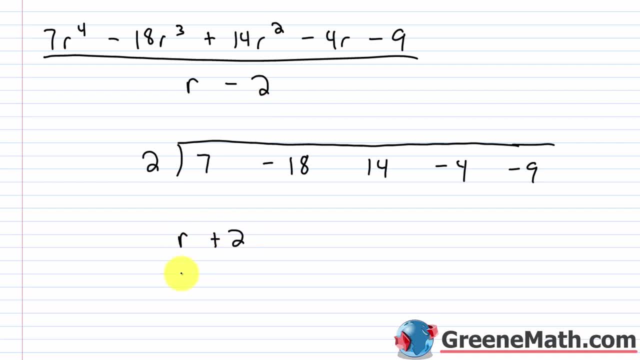 If I had something like r plus 2, I would rewrite this as r minus a negative 2.. And I'd be plugging in a negative 2 in that scenario. Very important, you understand what to plug in right here. Okay, Big source of. 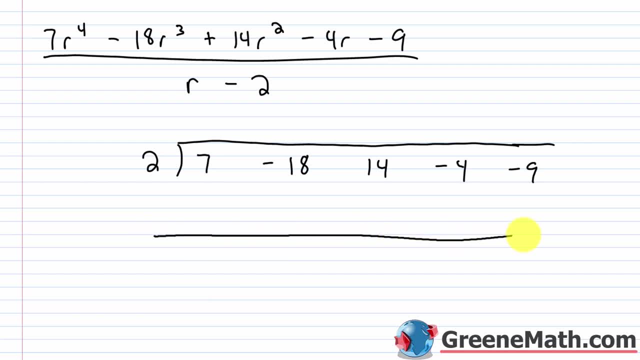 Confusion, All right, So let's go ahead and put a little bar here. We'll bring this down and we'll begin. So I'm not going to label row 1,, 2, and 3.. You should know this at this point. 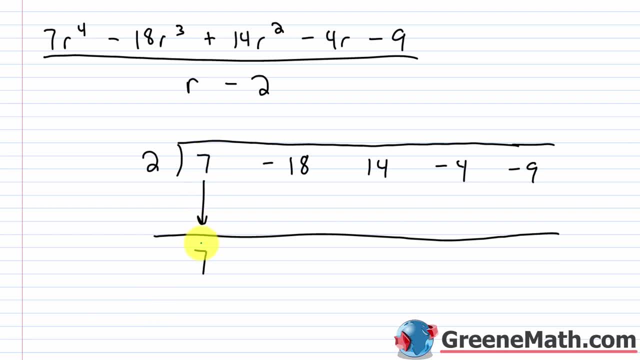 This is the third example. So after I bring 7 down to start it's multiply, then add, then multiply, then add. It just keeps going like that. So 2 times 7, I multiply, That's 14.. 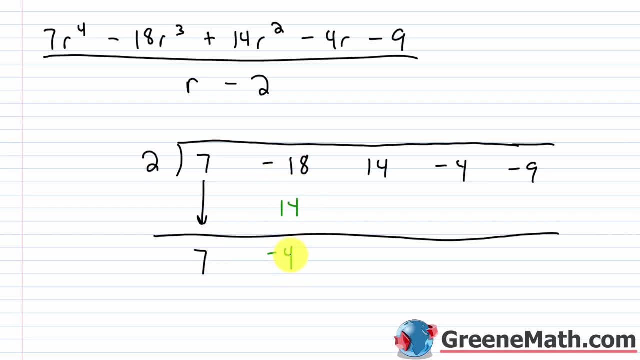 Then I add: Negative 18 plus 14 is negative 4. Then I multiply 2 times negative 4.. Negative 4 is negative 8. Then I add 14 plus negative 8 is 6. Then I multiply. 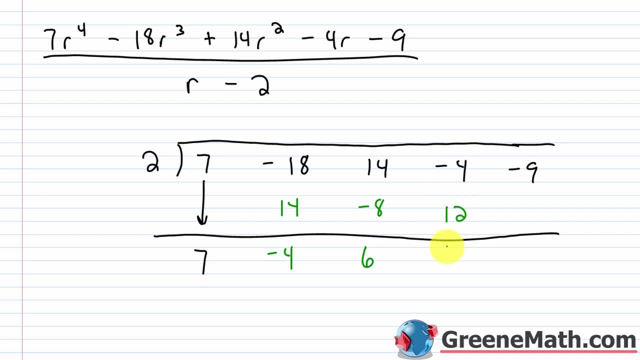 2 times 6 is 12.. Then I add Negative: 4 plus 12 is 8.. Then I multiply: 2 times 8 is 16.. Now I add Negative: 9 plus 16 is 7.. So again I can work left to right or right to left. 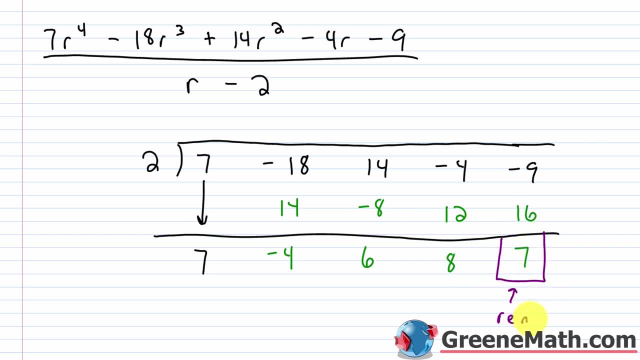 I know this is my remainder And I know this would be the constant. Then this would be the coefficient for r. so the first power, This would be the coefficient for r. the second power, Again, this is the velocity from the first to the second point into the denominator. 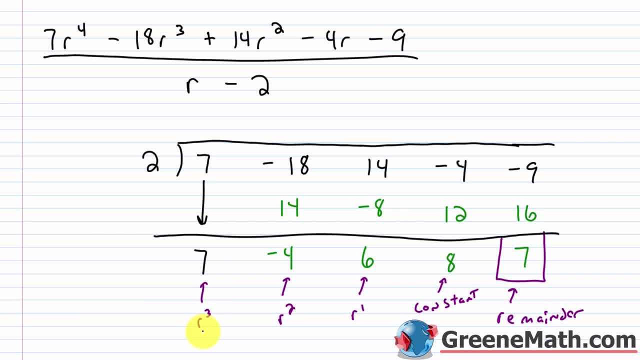 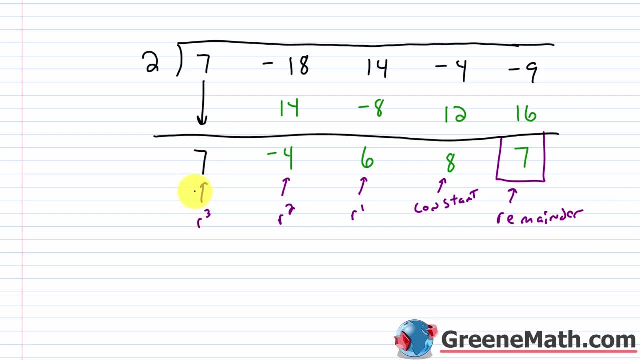 Then we have the return of 4 into r. Again, I get it right. Well, my result is my ratio, which means negative 21 to the 2 next step of my27.. The�� I can do, the power added 4 to the 16th. 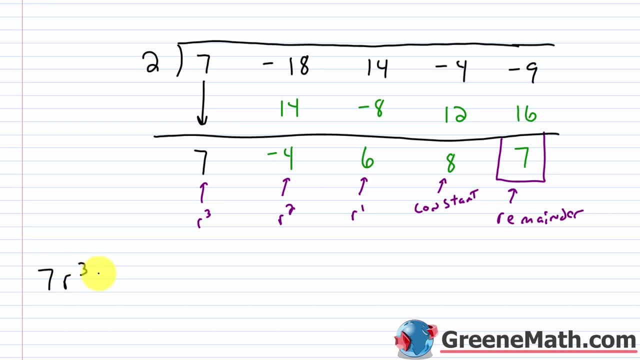 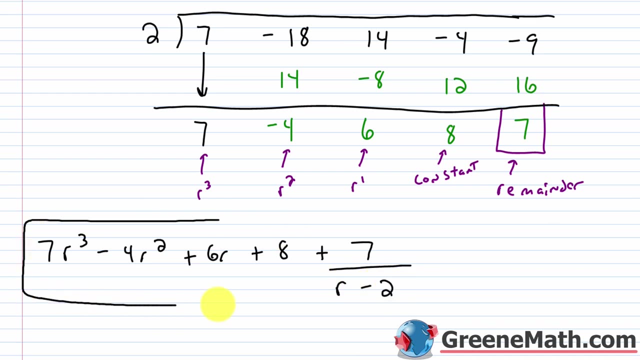 we would have 7r cubed, then minus 4r squared, then plus 6r, then plus 8, and then plus 7 over. our divisor is going to be r minus 2.. So this is your answer. here You end up with 7r. 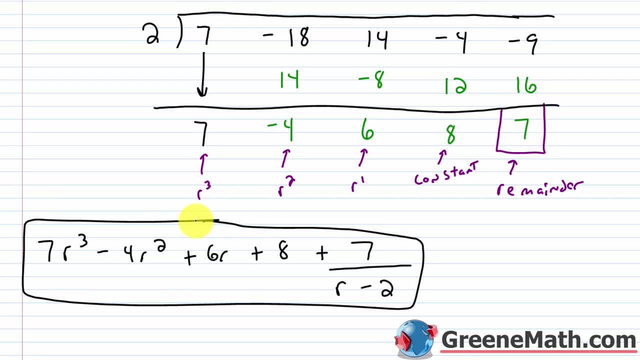 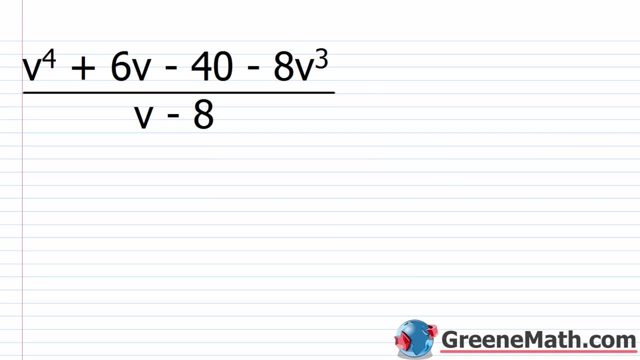 cubed minus 4r squared plus 6r plus 8 plus 7 over r minus 2.. All right, let's take a look at a couple more. So I have v to the fourth: power plus 6v minus 40 minus 8v cubed, This is over v. 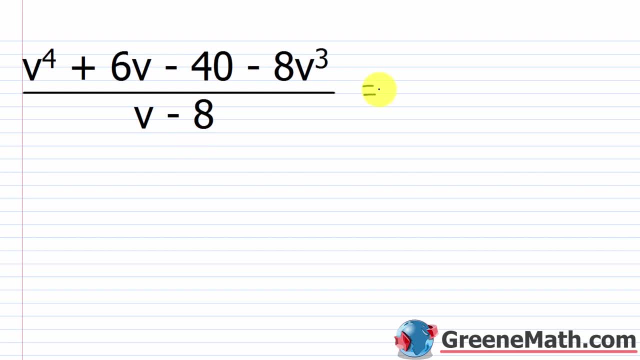 minus 8.. So again, let's put things in standard form and let's account for missing powers of the variable v. So if I start out with v to the fourth power, then minus 8v, cubed, I'm missing v squared. 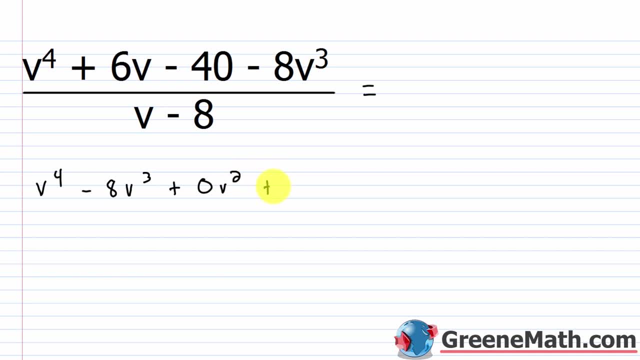 so let's put plus 0v squared, then plus 6v, then minus 40.. All right, then down here I have v minus 8. don't need to change anything there. and again, this follows the format of x minus k and. 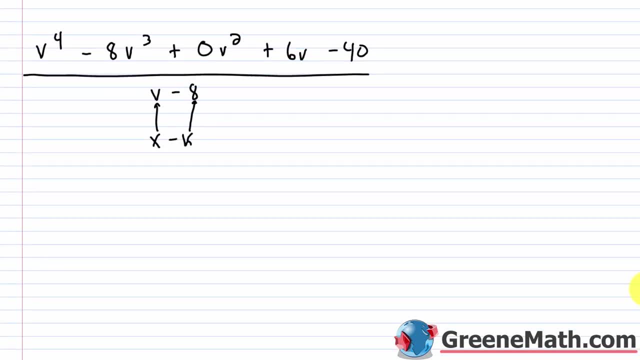 here x is just v and k is just 8. all right, so let's set everything up, and again i'm going to make a little long division symbol and underneath that long division symbol i'm going to take the numerical information here. so the coefficient for v to the fourth power is a 1. then i would go to: 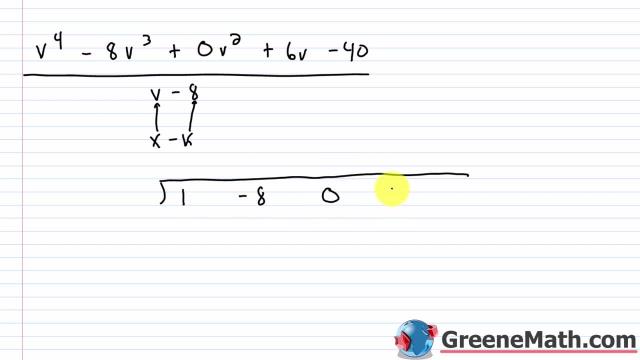 the next one, i have negative 8, then i'd have a 0, then a 6, and then finally a negative 40. now over here and again. if it's in the format of x minus k, this fits this perfectly. i just want this whatever k is. so in this case, this is going to be an 8 again. i'm going to say this one more time. if i 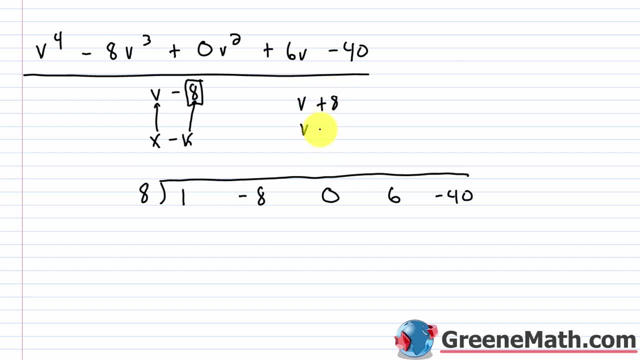 had something like v plus 8, i would rewrite it as v minus a negative 8. it would have a negative 8 out here. okay, again, most common mistake that i see. so i want to just keep saying it over and over again so that if you do make the mistake, you're like: oh, you warned me about that, and then you'll. 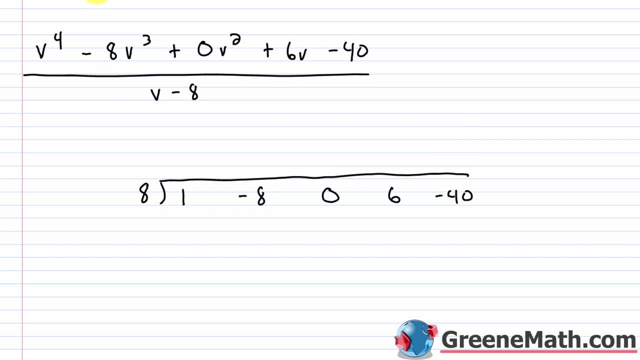 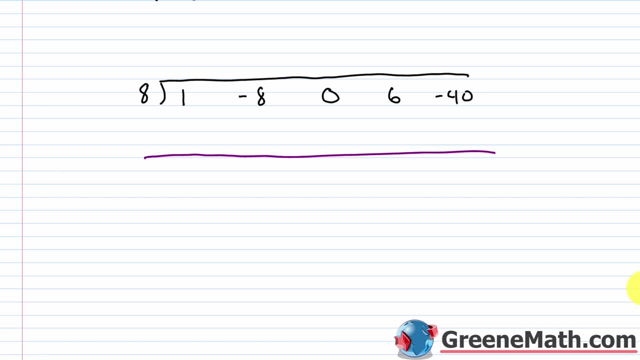 catch yourself and it'll stop you from making the mistake in the future. all right, so let me put a bar down here and again. it's a simple process. once you have everything set up, i bring this down, so bring down the 1, and i just multiply, then add multiply, then add multiply, then add. very, very simple so. 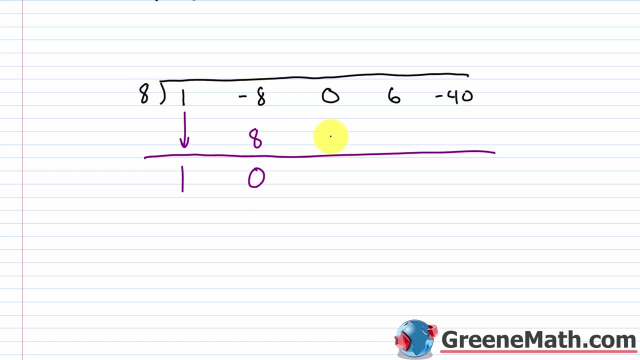 8 times 1 is 8. negative. 8 plus 8 is 0. 8 times 0 is 0. 0 plus 0 is 0. 8 times 0 is 0. 6 plus 0 is 6. 8 times 6 is 48 negative. 40 plus 48 is 8. 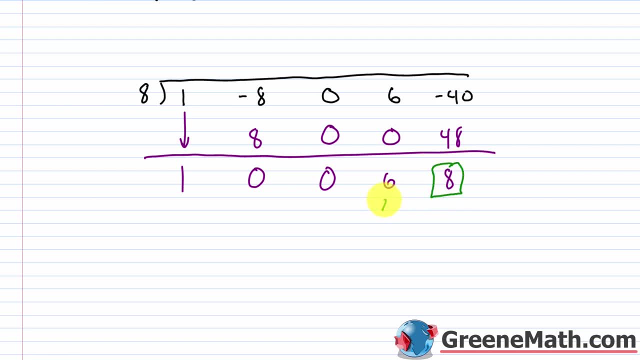 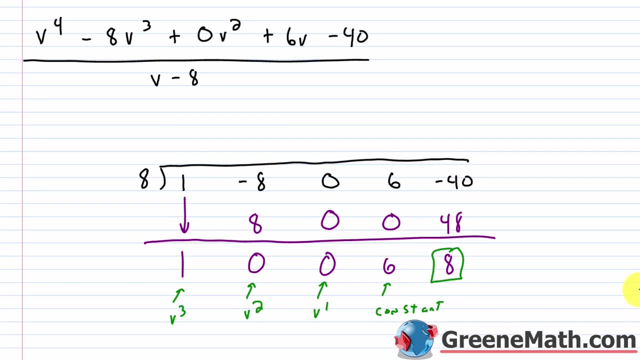 plus 9 is 8.. okay, now, what did i do? well, you add 6 times, now i do 0 and i also multiply till i get this bit of a problem. okay, this is the agreement v your. They're not superior in Capcom and what you mean here is v times 3 is kept and you are going to take aνε times three. 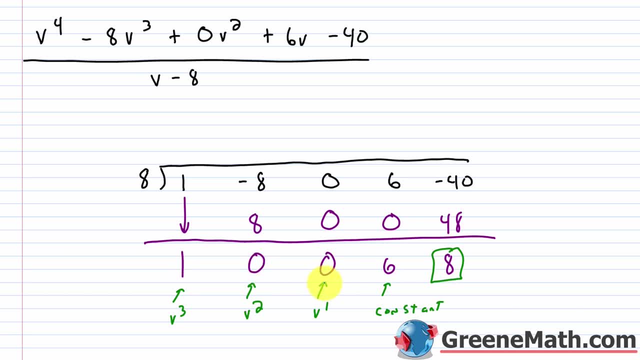 times exactly what they're going to do here. and then you're going to multiply the怎麼 it comes to value t. i will multiply the Uncle day two times three and you're gonna divide into half and so on. and again, if i look at my dividend, here it's got a degree of four, here i have a particular degree of three. 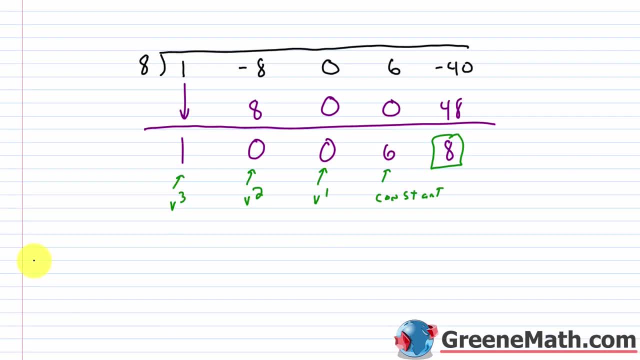 you know, so on and so forth. So to write our answer, I'd have one times V cubed or just V cubed. I'd have zero times V squared and zero times V. I don't need to write that. So then, 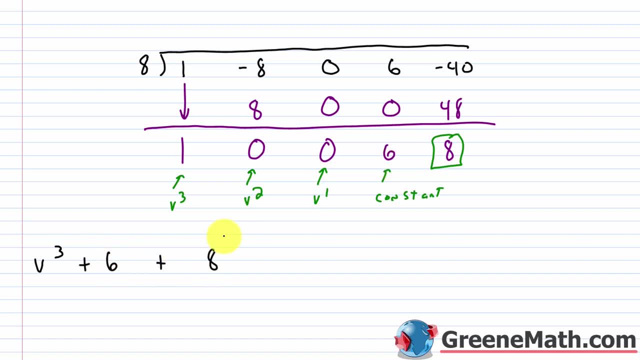 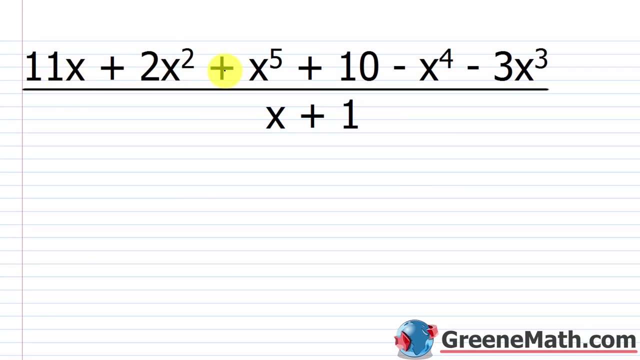 plus my constant six and then plus eight my remainder. Okay, Let me label that This is the remainder over my divisor, which was V minus eight, V minus eight, So V cubed plus six plus eight over V minus eight. All right, For the last problem, we have 11X plus two, X squared plus X to. 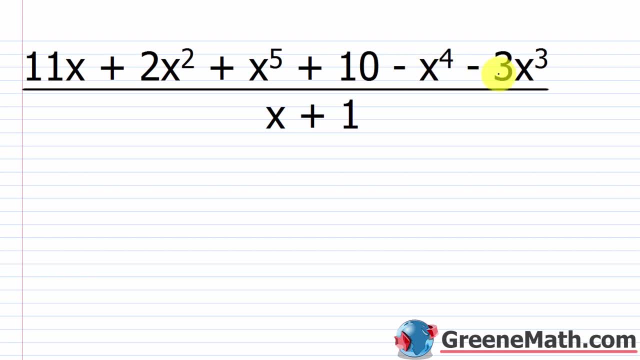 the fifth power plus 10, minus X to the fourth power, minus three X cubed, And this is over X plus one. So again, let's write it in standard form and let's account for any missing powers of X. So let's say that this is X to the fifth power. Now we're going to have minus X to the fourth. 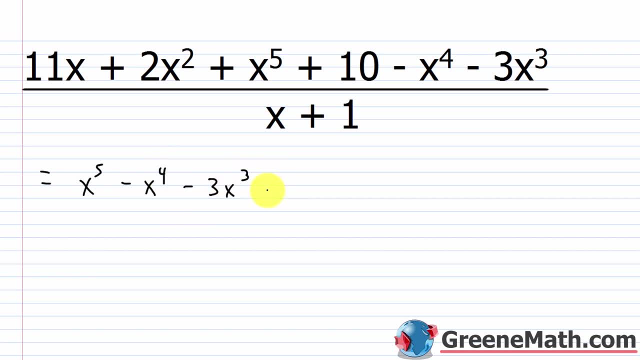 power, then minus three X cubed, And then we would have plus two X squared, And then we'd have plus 11X, And then, lastly, plus 10.. And this is over, We have X plus one. Now I'm going to go ahead and write X plus one as X minus a negative one. 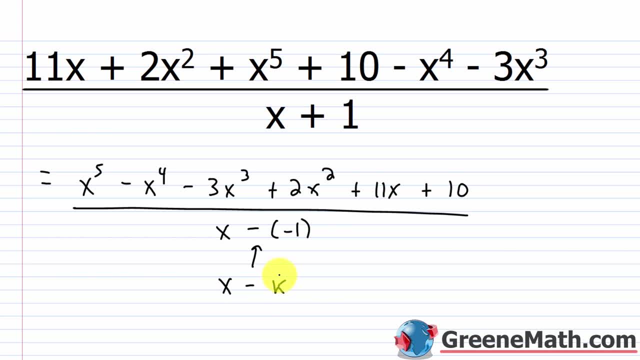 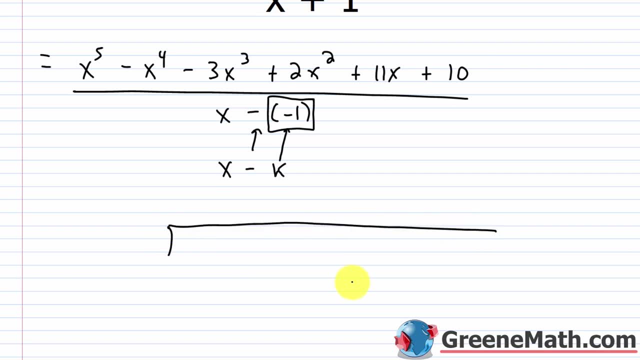 Again, I want this to be in the format of X minus K. Here K is going to be negative one. I'm going to make my little long division symbol. We're going to take the numerical information from the dividend. So I have a coefficient of X to the fifth power of one. 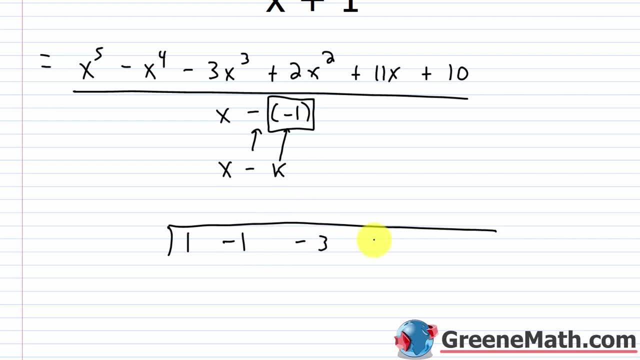 Then I would have negative one, then negative three, then two, then 11,, then 10.. Then when I think about K, again, it's negative one here because I wrote X minus a negative one. So this over here is going to be a negative one. Make sure you do that or you will get the wrong. 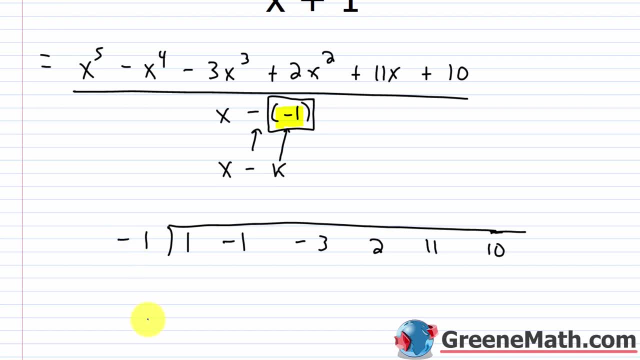 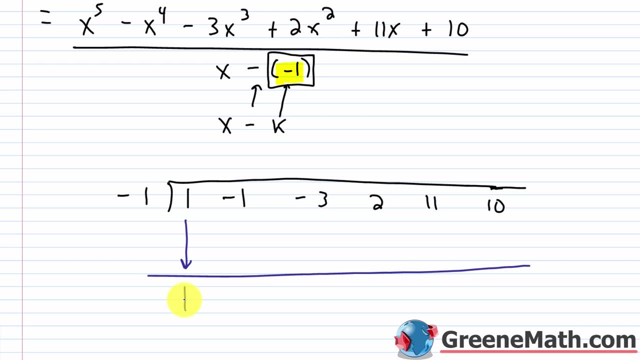 answer. Okay, Very important. All right, Let's put our bar down here and let's bring this down to begin. And again, we're going to multiply, then add, Multiply, then add, Multiply, then add. It's very, very simple, All right. So we start out with multiplication Negative one times one. 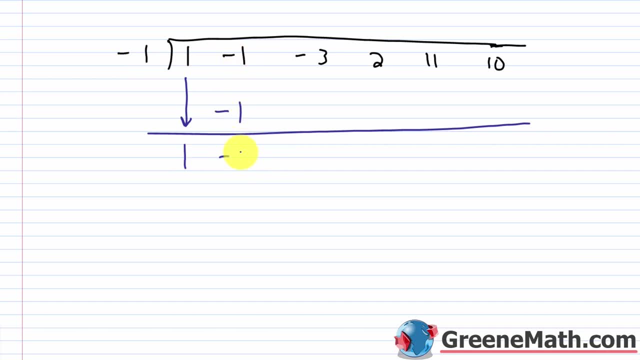 is negative one. Now we add Negative one plus negative one is negative two. Now we multiply Negative one times negative two is two. Now we add Negative three plus two is negative one. Now we multiply Negative one times negative one is one. Now we add Two plus one is three. 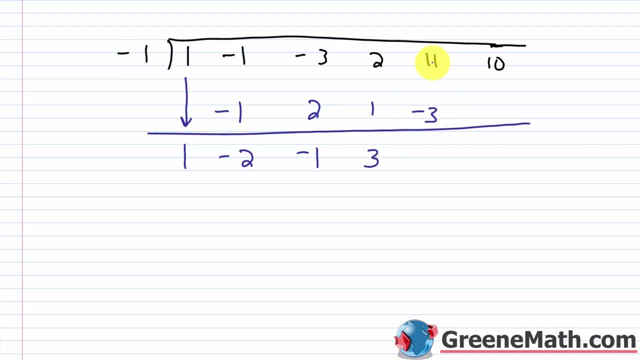 Now we multiply Negative one times three is negative three. Now we add 11 plus negative three is eight. Now we multiply Negative one times eight is negative eight. Now we add 10 plus negative eight is two. So we're done. We know that this is our remainder. 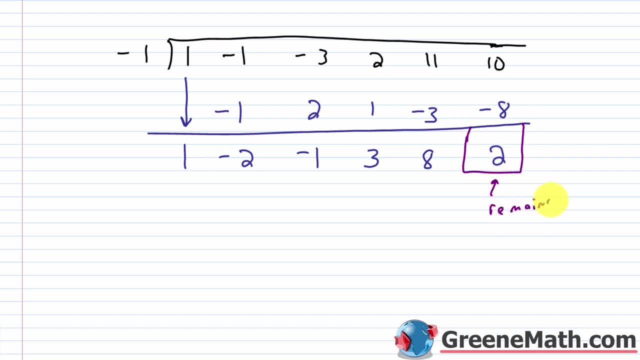 This is our remainder, This is our constant, This is our coefficient for X to the first power, our coefficient for X squared, our coefficient for X cubed and our coefficient for X to the fourth power. So what we would have as our answer is one X to the fourth power, just X to the fourth power. 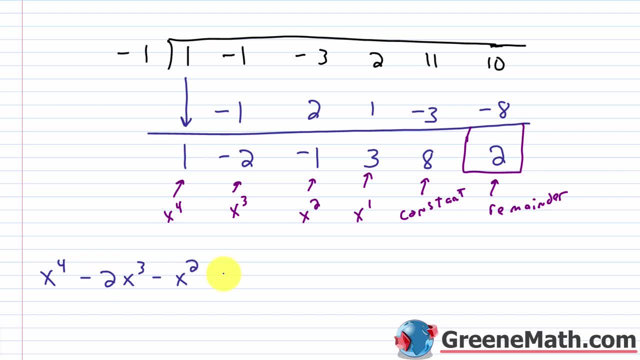 minus two, X cubed minus X squared plus three, X plus eight, then plus You'd have two over. Remember, your divisor here was X plus one. We wrote it as X minus a negative one, but originally it was X plus one, So two over X plus one. So this right here will be your answer. 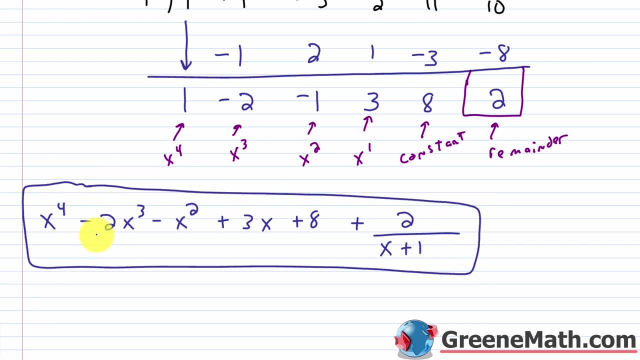 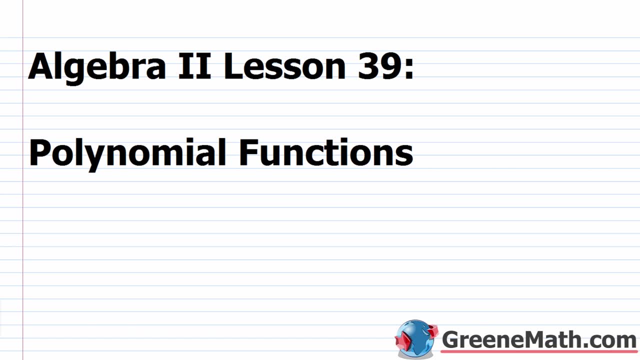 X to the fourth, power minus two, X cubed minus X squared plus three, X plus eight plus two over X plus one. Hello and welcome to Algebra 2, Lesson 39.. In this video, we're going to learn about polynomial. 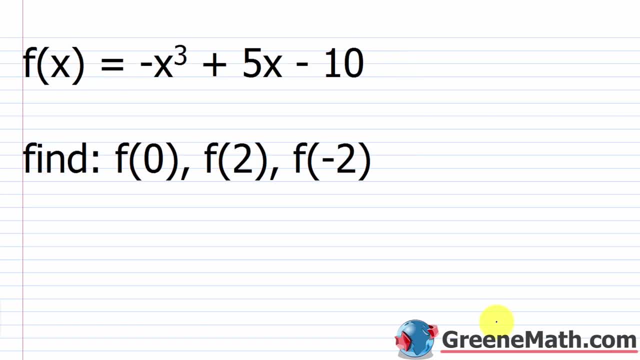 functions. So essentially what we're going to look at in this lesson, we're going to look at polynomial functions and operations with polynomial functions. So I want to just start out with a polynomial function. We have F of X is equal to. we have negative X cubed plus five, X minus 10.. 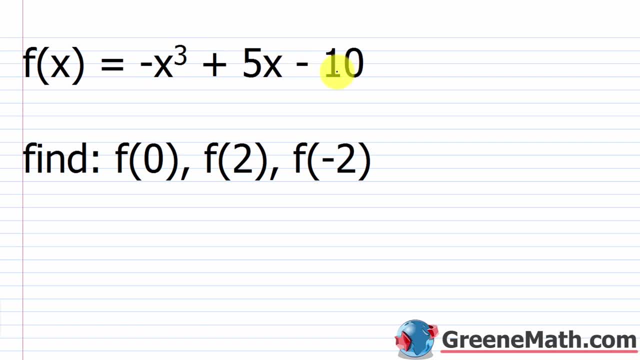 Now, in a previous lesson in Algebra 2, I taught you about function notation. So if I ask you to find F of zero, F of two or F of negative two, at this point you should be able to do that. 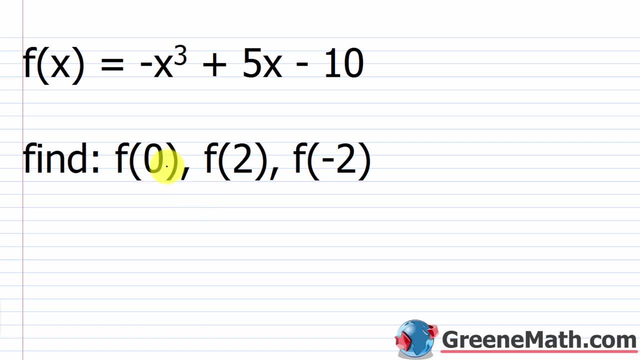 Essentially what I'm doing. if I ask for something like F of zero, I'm saying: what is the function's value if the independent variable X is zero? So I would have negative. I'd plug in a zero for X and that would be cubed plus five times. I'd plug in a zero for X. 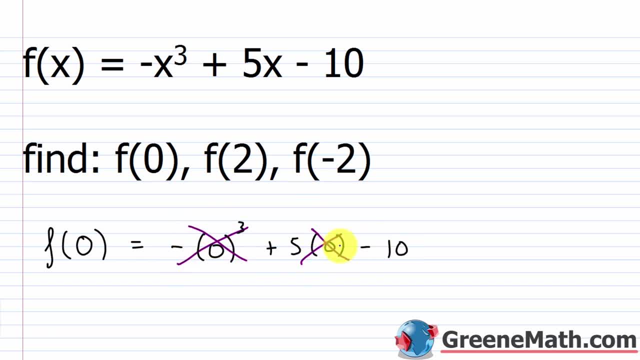 then minus 10.. So we could see that these two would be zero. So I'd have zero plus zero, which is zero, then minus 10,, which is just negative 10.. So F of zero is negative 10, or the function's value. 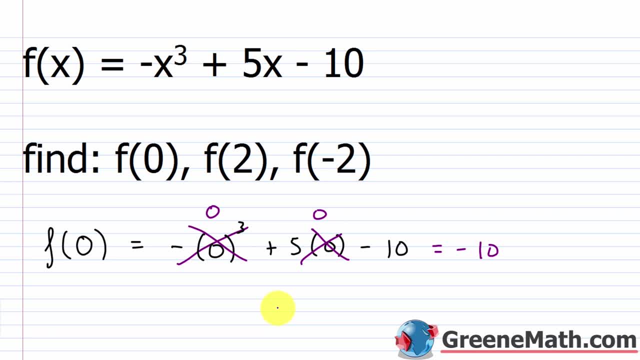 when the independent variable X is zero is negative 10.. All right, what if we did F of two? Okay, F of two, Same concept. What I'm going to do is I'm going to replace every X with a two. 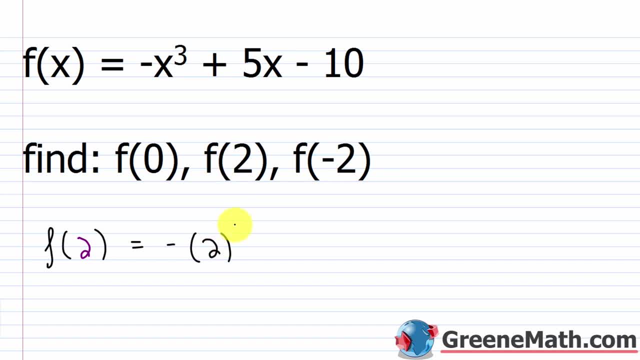 So negative. and then I have a two being plugged in for x. this is cubed, then plus 5 multiplied by again. 2 is plugged in for x, then minus 10. so 2 cubed is 8. I'd want the opposite of. 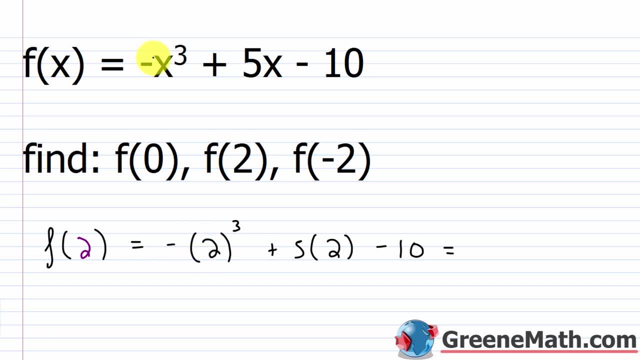 that. notice how the negative is not inside of parentheses, it's outside here. okay, so the opposite of 8 would be negative 8. then plus we have 5 times 2, which is 10. then we have minus 10. so we know 10 minus 10 is 0, so that's. 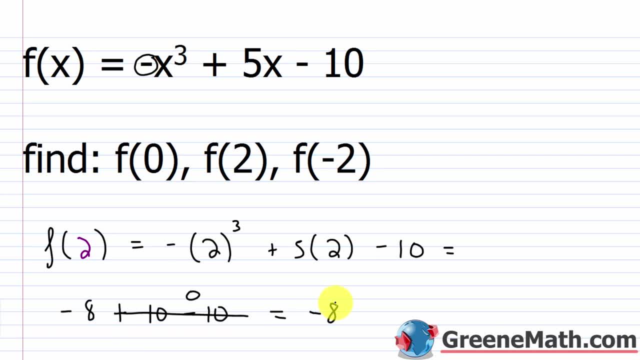 basically cancelled. we're left with just negative 8 there. so f of 2 is negative 8. all right then. the last one we wanted to look at is f of negative 2. so again, I'm just going to plug in for my variable X: so negative, then we plug. 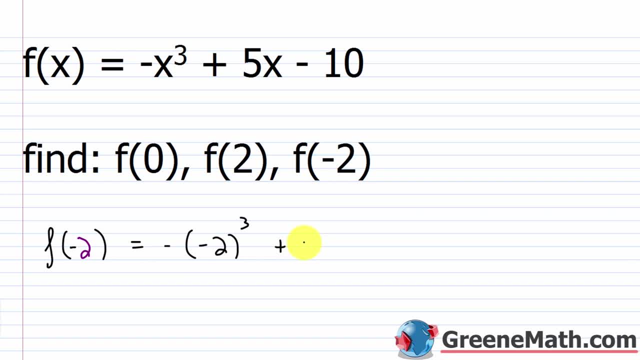 in a negative 2 and that's cubed. then plus we have 5 times: plug in a negative 2 for X, then minus 10. so negative 2: cubed is negative 8. again this negative 2 is negative 8. so we plug in a negative 2 for x, then minus 10. so negative 2: cubed is negative 8. again this negative. 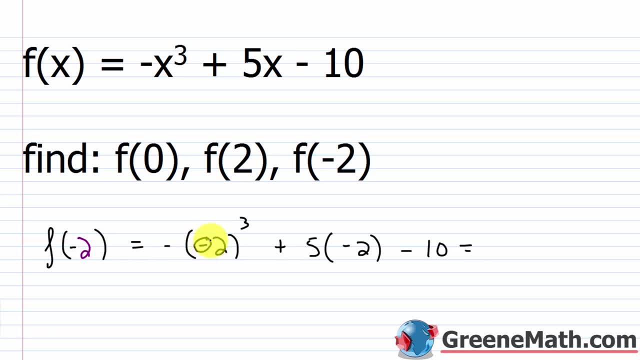 here is inside the parentheses, so it's included. negative 2 times negative 2 is 4. 4 times negative 2 is negative 8. so I would have the opposite of negative 8 which is positive 8. then we have 5 times negative 2, which is negative 10. then 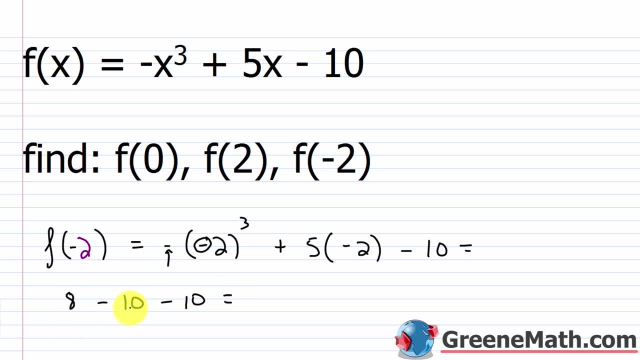 minus 10. so we would have 8 minus 10, which is going to give me negative 2, and the negative 2 minus 10, which is going to give me negative 12. so f of negative, 2 is negative, 2 is going to be negative 12, all right, so let's look at one more just. 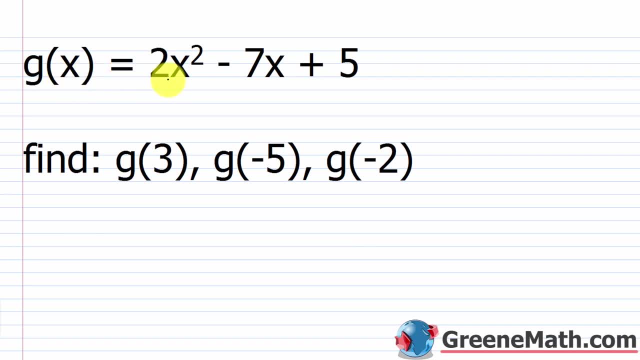 as a review. if I had something like G of X equals 2x squared minus 7x plus 5, and I wanted to find G of 3, G of negative 5 and G of negative 2, what would I do again? I'm just going to be plugging in for the variable. it's not very hard if I 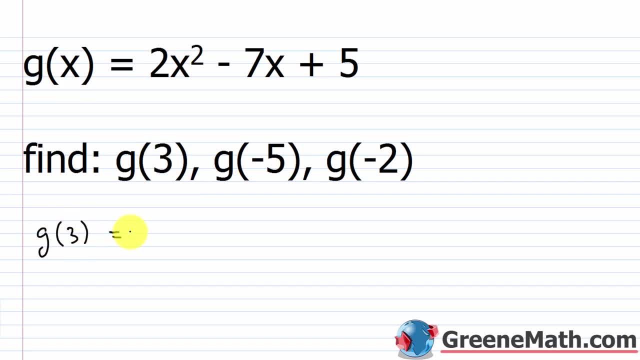 want G of 3. that's telling me just to plug in a 3. everywhere I see an X, and so 2 times we'd have a 3 plugged in there. that's squared minus 7 times. plug in a 3 for X here. then plus 5, 3 squared is 9, 9 times 2 is 18, so this would be 18. 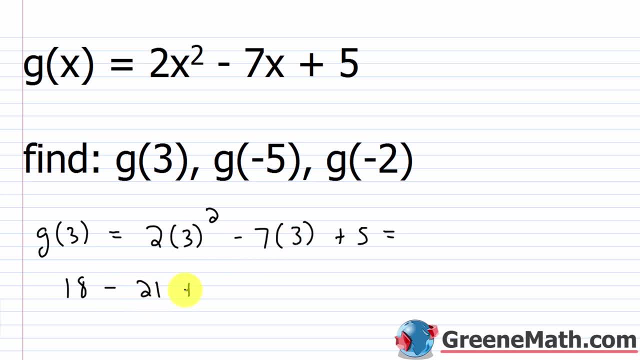 then minus 7 times 3 is 21, then plus 5. if I take 18 and I subtract away 21, I get negative 3. negative 3 plus 5 is positive 2. all right, the next thing I want to look at is G of negative 5. again, all I'm doing is I'm plugging in a 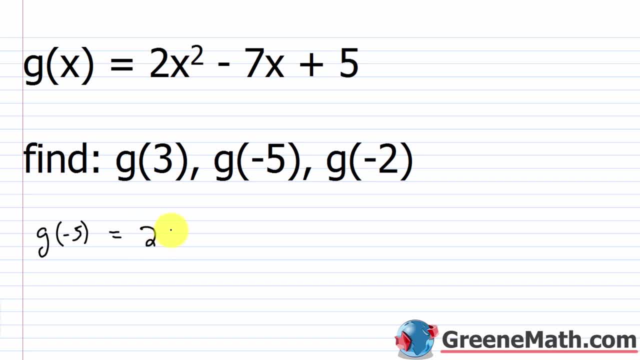 negative 5 for my variable X, so 2 times. plug in a negative 5 for X. that's squared minus 7 times. plug in a negative 5 for X plus 5 negative 5 squared is 25. 25 times 2 is 50. so this would be 50 negative 7 times negative. 5 is positive. 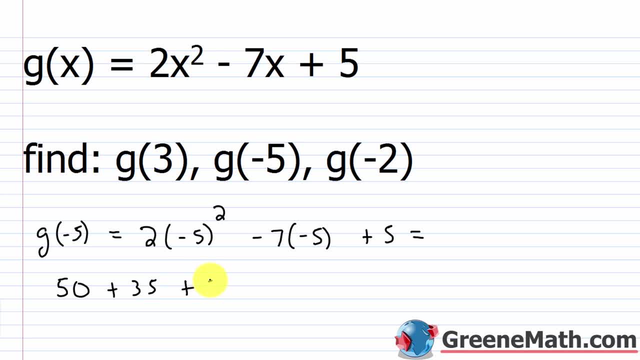 35, so plus 35, and then plus 5, so 50 plus 35 is 85, 85 plus 5 is 90. all right then. 1, we want to find G of negative 2, a G of negative 2, so all I'm going to do once. 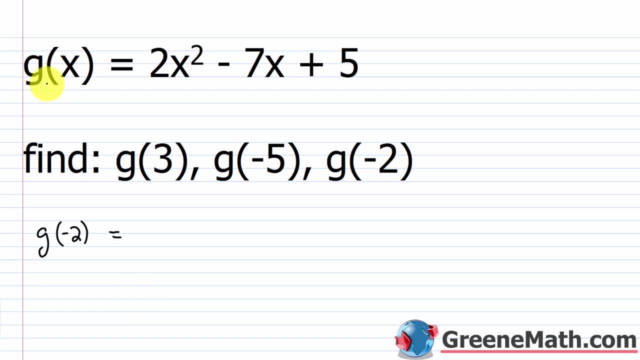 again, super, super simple. if I have G of negative 2, I plug in a negative 2. everywhere I see an X. so I have 2 times negative 2. plug that in for X. that's squared minus 7 times. plug in a negative 2 for X plus 5. very, very easy. negative 2. 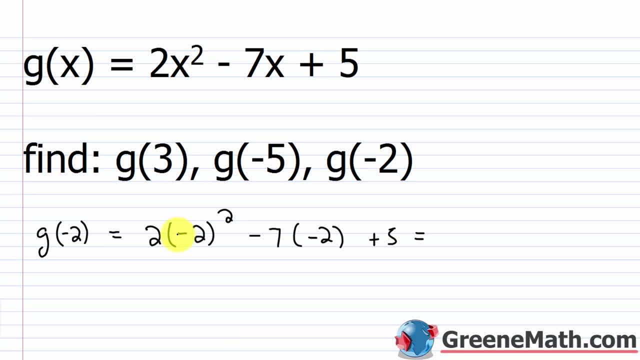 squared again. the negatives involved in the equation is so that would be 4 4 times 2 would be 8, so you'd have 8 negative 7 times negative. 2 is positive 14, so plus 14, and then plus 5, so 8 plus 14 is going. 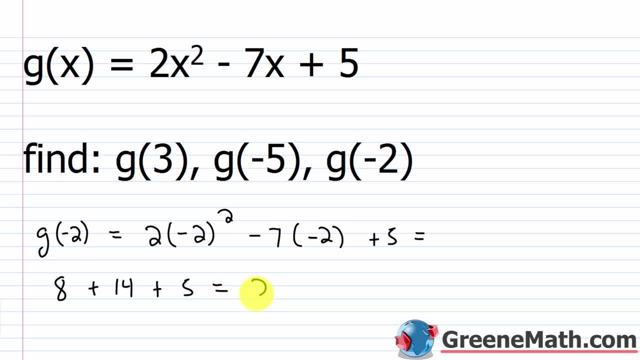 to give me 22. then 22 plus 5 is 27, so pretty easy overall, but something I wanted to do a refresher on before we started kind of going to the next level. in a moment we're gonna look at operations with polynomial functions. all right, so the very first thing we're gonna do is we're gonna look at the 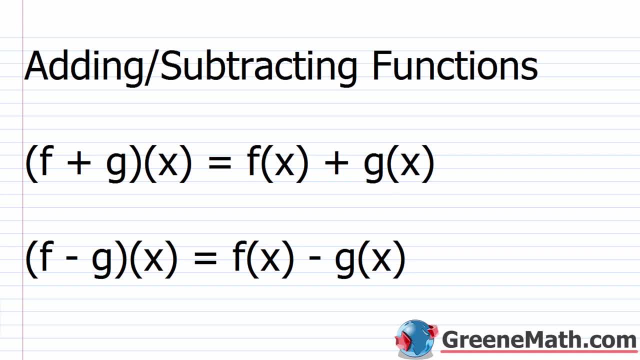 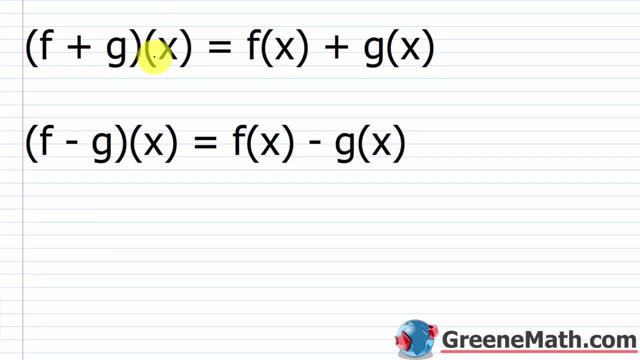 polynomial functions, and we're gonna learn how to do is adding and subtracting functions. okay. so if you see something like F plus G of X with this notation here, all this is telling you to do is take F of X and add G of X. okay so. 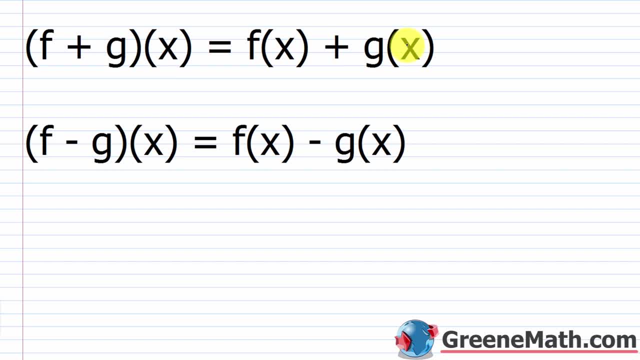 all you're gonna be doing is basically combining like terms. it's just like if I added two polynomials together, it's no more difficult. okay, you've just got to get used to the notation. it's the same thing. if I see something like F minus G of X, this is F of X minus G of X. now it's gonna get more complex. 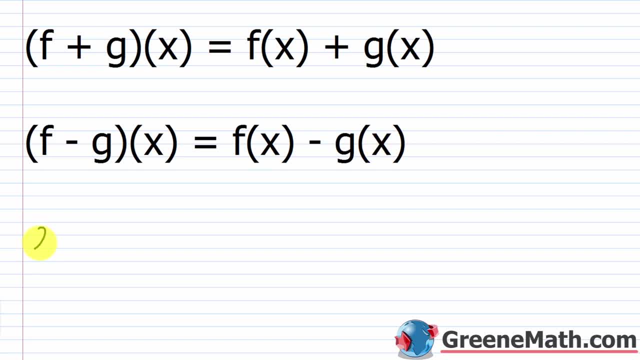 because they're gonna ask you for stuff like this. they're gonna say F plus G of, let's say, 2. all I'm doing is I'm finding the function F of X plus the function G of X and I'm gonna take that result and I'm going to plug in a 2 everywhere. 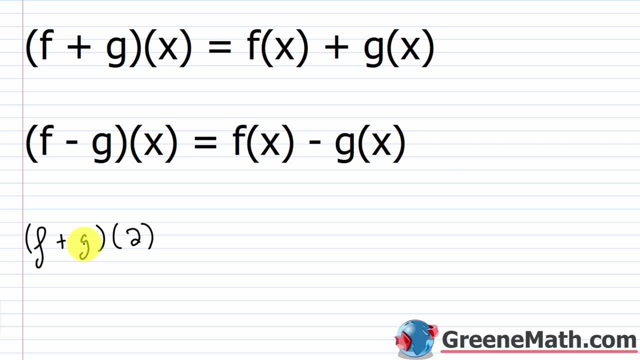 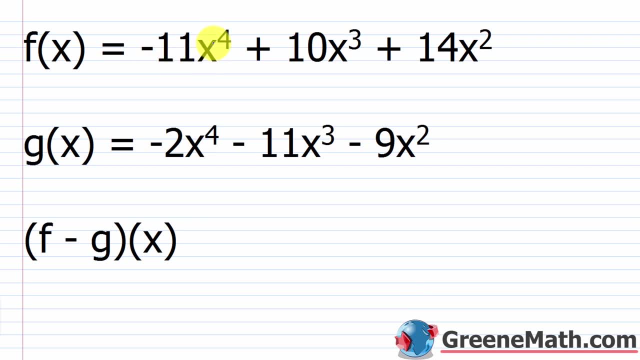 there's an X and I'm gonna find out what that value is. okay, that's all this is asking for. okay, so let's take a look at an example. so suppose you see something like: F of X equals negative 11 X to the fourth power, plus 10 X cubed plus 14 X. 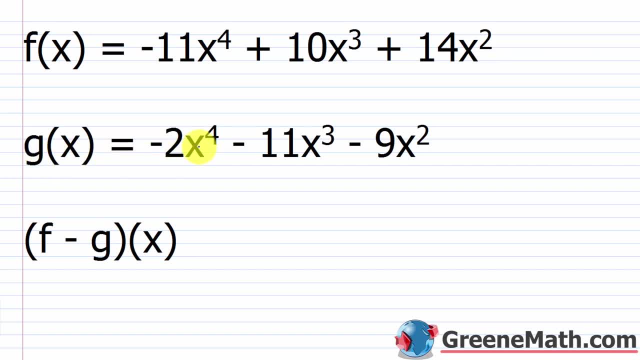 squared and you see G of X is equal to negative 2 X to the fourth power minus 11 X cubed minus 9 X squared. now the problem we get: we're told to do F minus G of X. so all I'm gonna do this is super, super easy. the order matters: F comes. 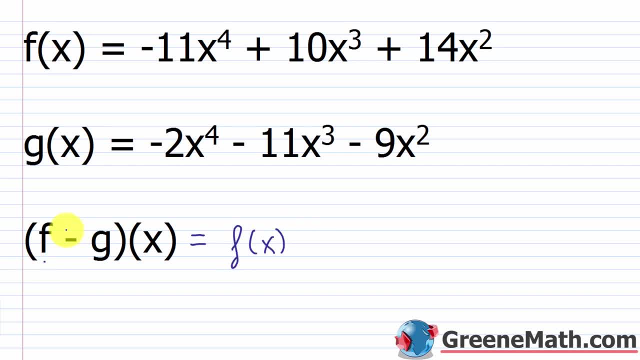 first. so I want F of X, then minus G of X. okay, so what's that going to be equal to? well, if I have my function F of X, it's what it's negative: 11 X to the fourth power, plus 10 X cubed, plus 14 X squared. now, if I subtract away my function G of X, remember if I'm 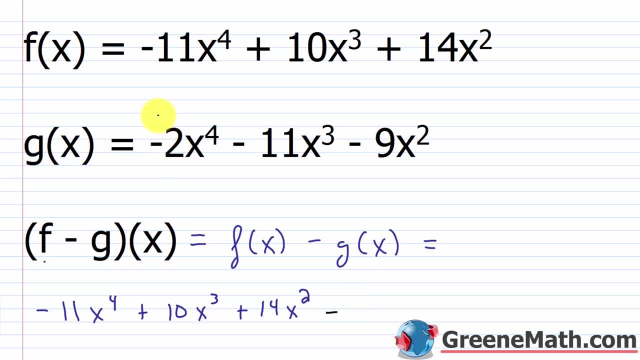 subtracting something away. we've got to put it inside of parentheses, so this whole thing needs to be subtracted away. don't make the mistake of just subtracting away the first kind of term. there you want minus and then, inside of parentheses, you want negative. 2 X to the 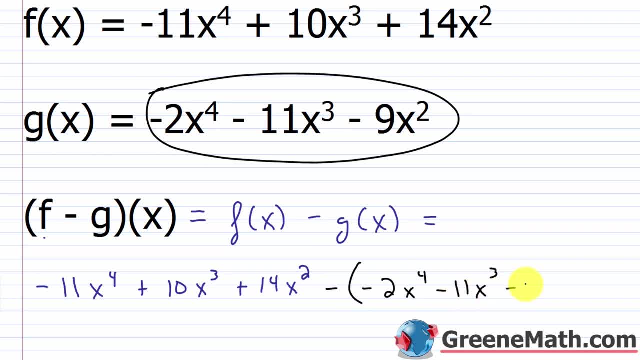 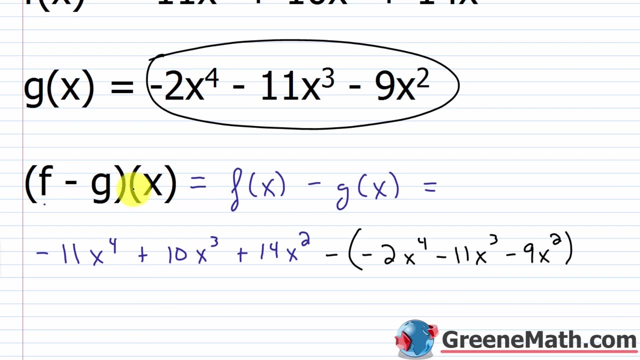 fourth power: minus 11 X cubed, minus 9 X squared with subtraction. remember, the order always matters. so I have F of X here and then I have G of X here. okay, very important. if this was G minus F of X, the order would be flipped, alright, so 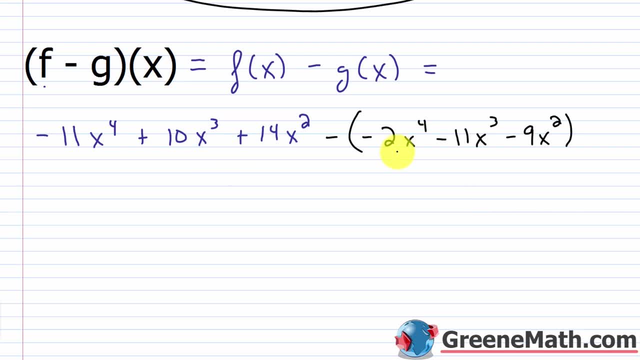 once we've kind of set this up, we're gonna have to do a little bit of a up. it's no different than just subtracting polynomials. The only thing you really have to get used to is just the notation involved. Once you get used to what it's telling you to do. 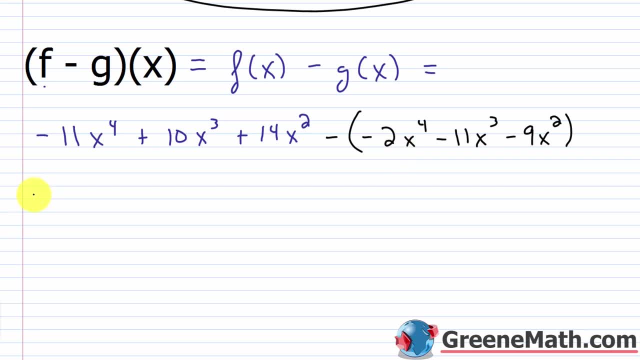 the actual operation itself is quite simple, So I would rewrite this as negative: 11x to the fourth power plus 10x cubed, plus 14x squared. I would distribute this kind of negative to each term. So minus a negative 2x to the fourth power would be plus 2x to the fourth power. 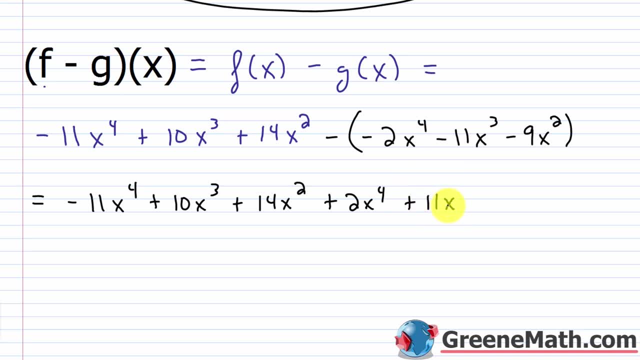 Minus a negative 11x cubed would be plus 11x cubed, And then, lastly, minus a negative 9x squared would be plus 9x squared. So all I need to do now is just combine like terms. 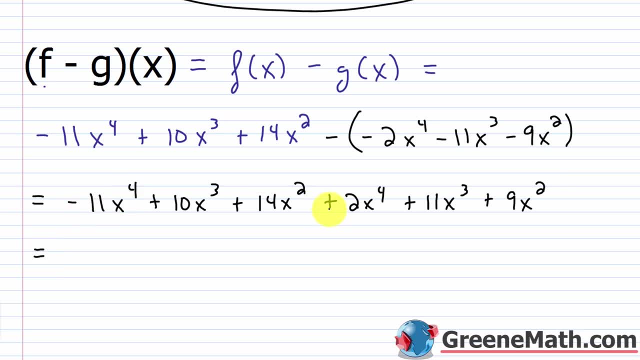 and I have my answer. Negative 11x to the fourth power plus 2x to the fourth power would give me negative 9x to the fourth power. Then I would have 10x cubed plus 11x cubed. That would be plus 21x cubed. Then I would have 14x squared plus 9x squared. That would give me. 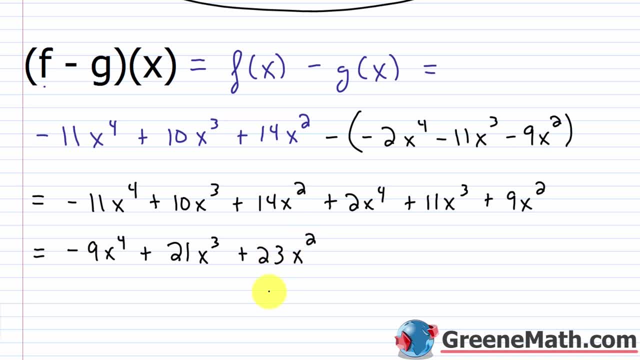 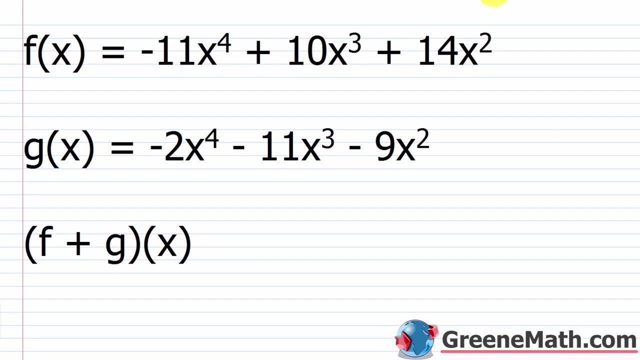 plus 23x squared. So this is my answer here. This is f minus g of x. Okay, that's the result that you get. It's negative 9x to the fourth power plus 21x cubed, plus 23x squared. All right. 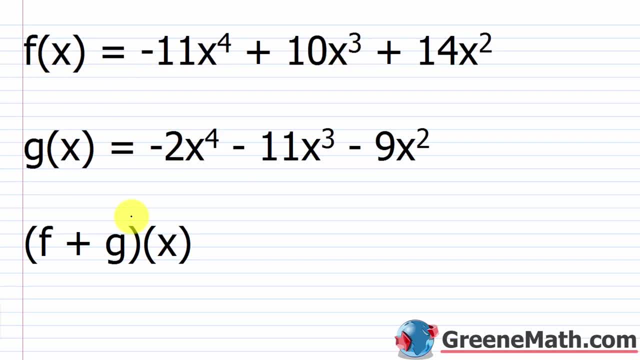 so let's say, we had the same function for f of x, the same function for g of x, But now we've changed the problem to f plus g of x. So we want to find this. So now we're just going to add f of x plus g of x. Okay, and with addition the order does not. 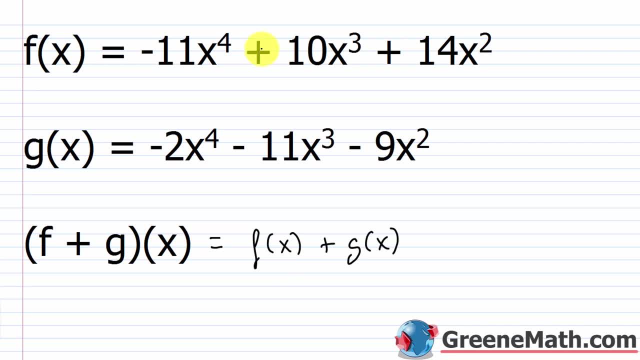 matter. So I could put f of x first, or I could put g of x first, I would get the same answer, right, It would not matter With subtraction, the order does matter, Okay, so that's where you've got to pay close attention. So I'm going to start out by writing my 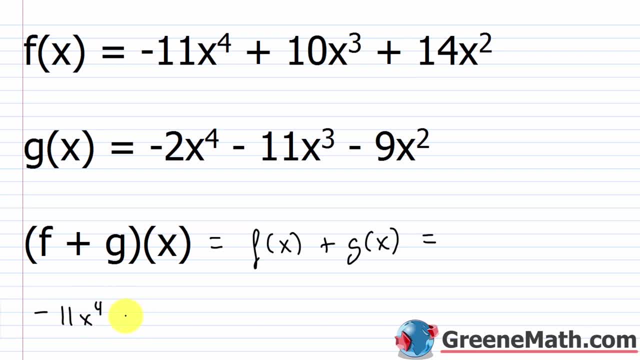 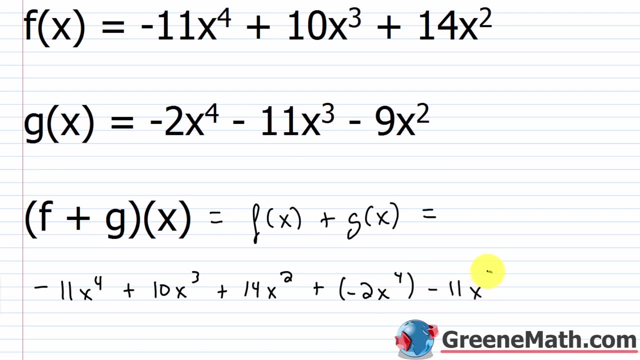 f of x. So this is negative 11x to the fourth power, plus 10x cubed, plus 14x squared. Then I'm going to add to this, I'm going to have negative 2x to the fourth power and then minus 11x cubed and then minus 9x squared. So what would the result here be? 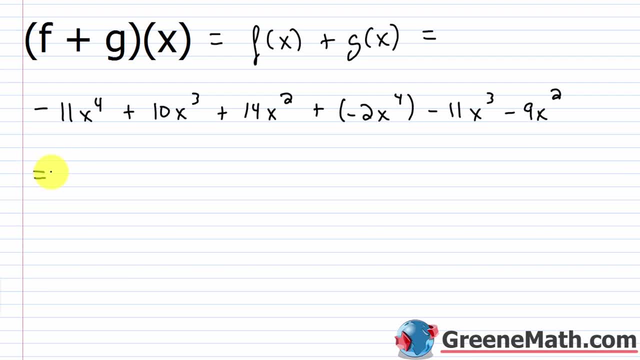 Well, again, I'm just going to combine like terms, just like I would if I was adding polynomials Negative 11x to the fourth power plus negative 2x to the fourth power is negative 13x to the fourth power If I have 10x cubed minus 11x. 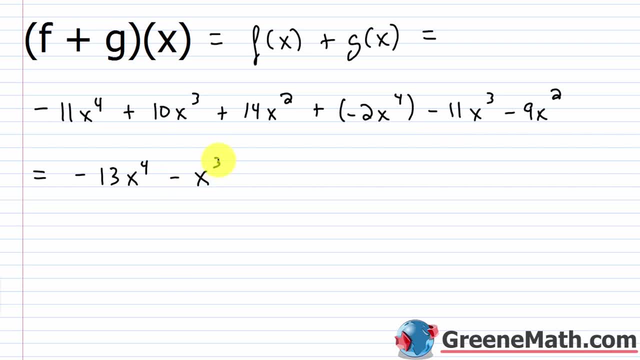 cubed, that's going to give me negative x cubed. And then, lastly, if I have 14x squared minus 9x squared, that's going to give me plus 5x squared. So I'm going to end up with negative 13x to the. 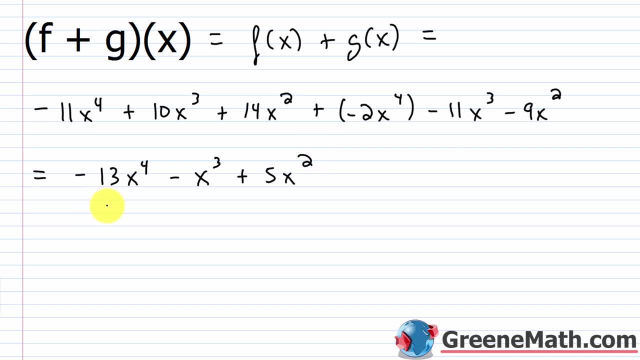 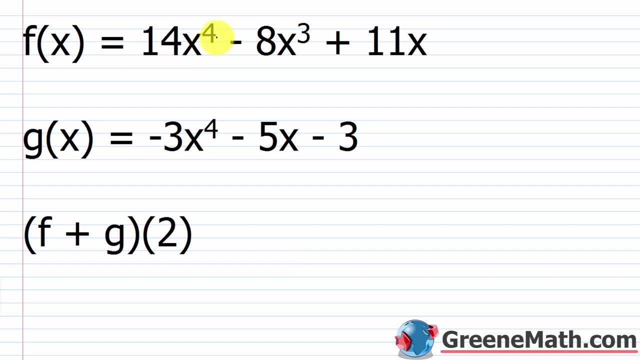 fourth power minus x cubed plus 5x squared All right. so let's kind of take things up just a notch And let's say we had f of x equals 14x to the fourth power, minus 8x cubed plus 11x. 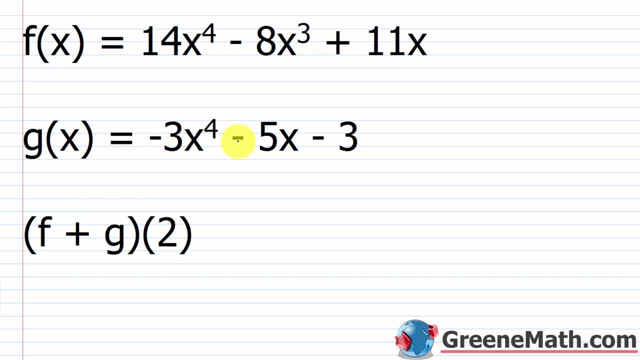 And we have: g of x is equal to negative 3x to the fourth power, minus 5x minus 3.. Let's suppose you see something like this: f plus g of 2.. So again, this notation is just something you have to get. 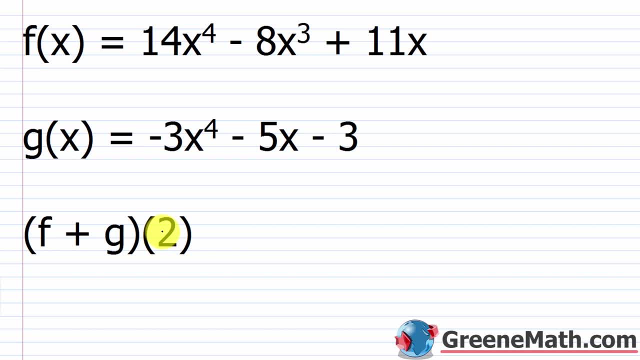 used to. Let me think of what in the world does that mean? What it means is I'm going to find f of x plus g of x, And when I get that result, I'm going to have to find f of x plus g of x. 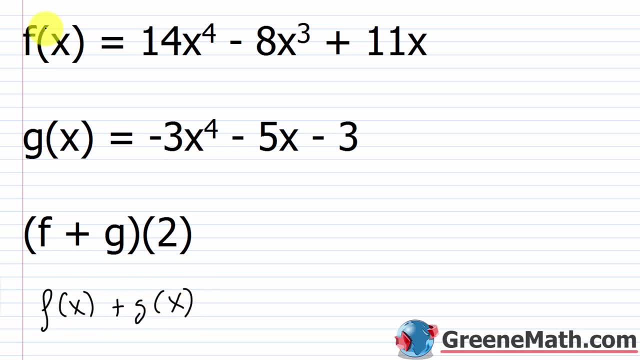 And when I get that result, I'm going to have to find f of x plus g of x. And when I get that result result I'm just going to plug in a 2 for x. Another way to explain it is: I could find f of 2. 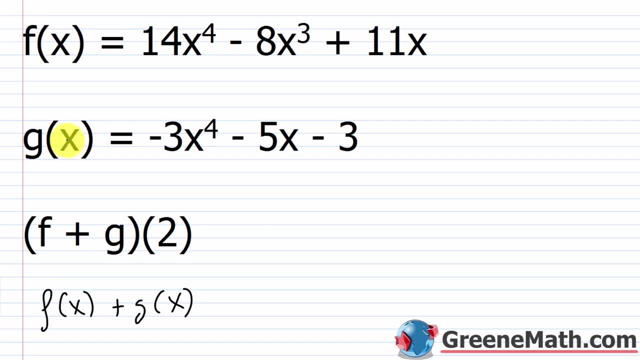 and g of 2, and then I could just sum those together And it's just two different ways that you could achieve this, and I'm going to do both for you. So the first way I'm going to do this is I'm going to find f of 2 plus g of 2, okay, So to do that, f of 2 would be what It would be 14. 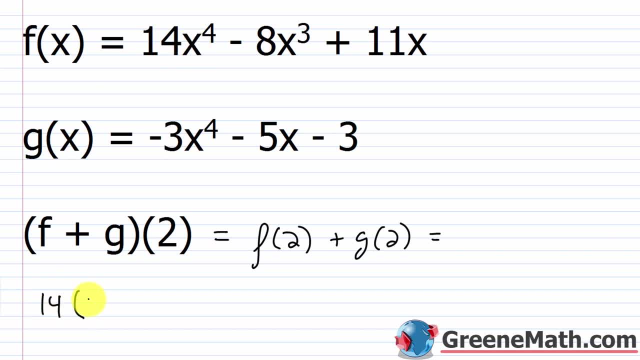 times I'd plug in a 2 for x, so 2 to the fourth power minus 8 times. I'd plug in a 2 for x, so that's cubed plus we'd have 11 times. plug in a 2 for x, Then plus. Now I want g of 2.. 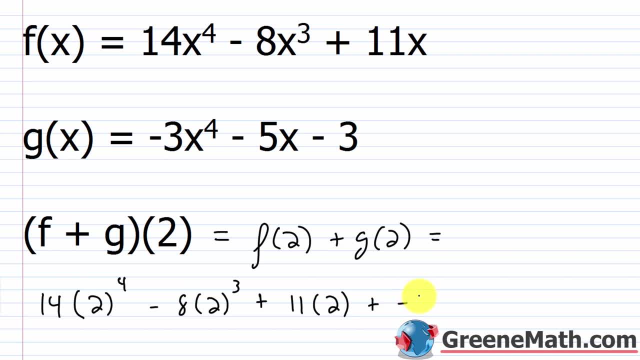 So g of 2, I'm plugging in a 2 for x. So negative 3 times you'd plug in a 2, and that would be to the fourth power minus 5 times. plug in a 2,. 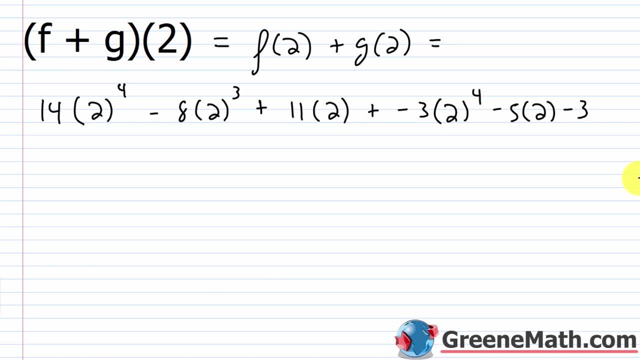 and then minus 3.. All right, so what does this give us? 2 to the fourth power we know is 16, then 16 times 14 is 224.. Then we have minus 2: cubed is 8,, 8 times 8 is 64,, so 64. 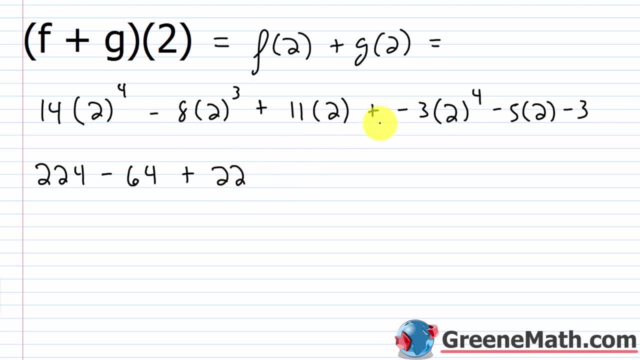 Then plus 11 times 2 is 22.. Then we have 2 to the fourth power. we know that's 16, you multiply that by negative 3, that's going to give you negative 48, so let's put minus 48.. 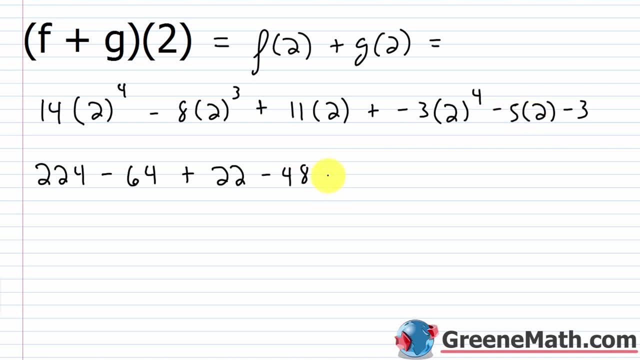 Then here we have negative 5 times 2,, that's negative 10, so negative 10, and then minus 3.. So now we're just going to work left to right: 224 minus 64 would give us 160, plus 22 would be 182, minus 48 would be 134, minus 10. 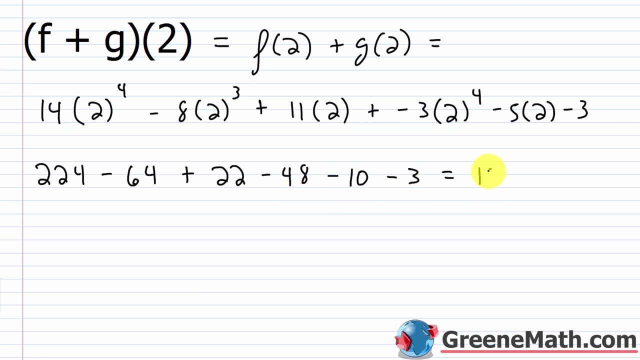 would be 124, then minus 3 would be 121. So this is f plus g of 2.. Now the other way we could have got this- just remember you got 121. Let's erase this. The other thing we could have done is we could have first added f of x plus g of x, If I have. 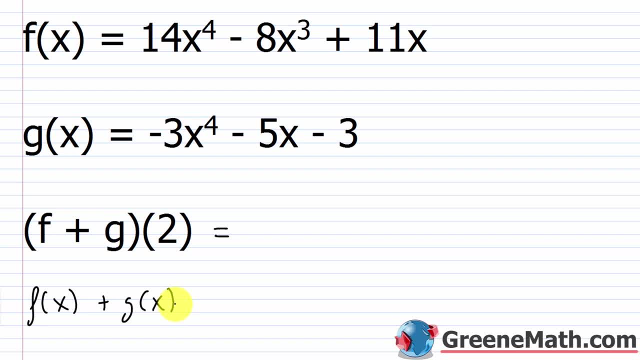 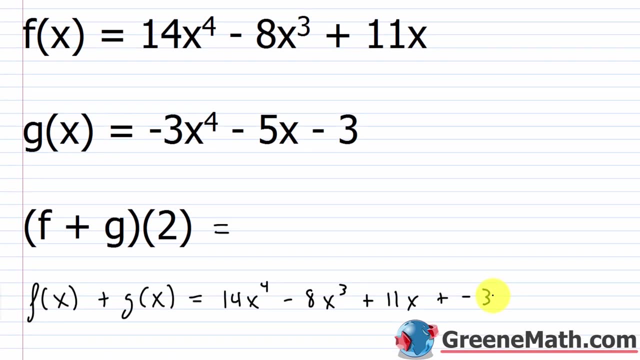 f of x plus g of x. this is going to be equal to: we'd have 14x to the fourth power minus 8x, cubed plus 11x, and then plus g of x, which is negative 3x to the fourth power minus 5x minus 3.. 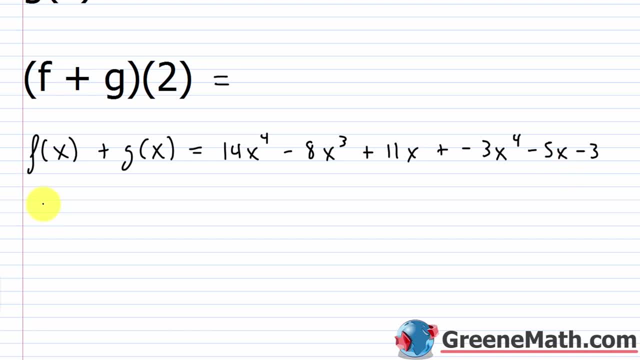 Again, all I'm looking to do is just combine like terms here. So I put: equals 14x to the fourth power, minus 3x to the fourth power is 11x to the fourth power, Negative 8x. cubed nothing to combine. 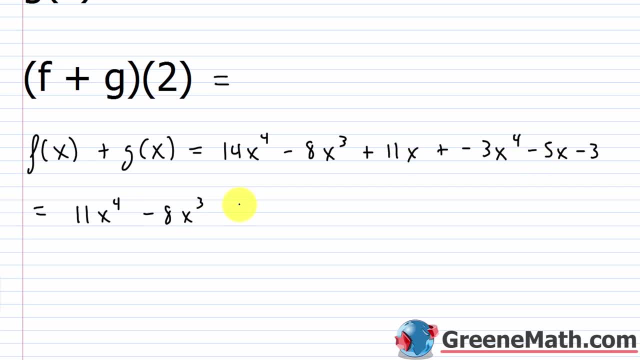 with that, I have 11x and minus 5x. that's positive 6x, and then I have minus 3.. So once I have this result, what I'm looking for is to substitute a 2 in everywhere I see an x, So I'd. 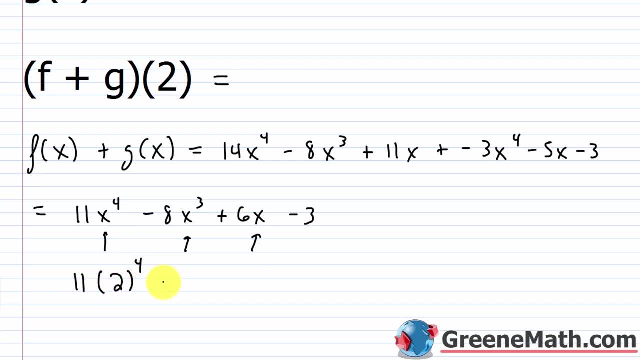 put a 2 in for x, so 2 to the fourth power minus 8 times. plug in a 2 in for x, so 2 raised to the third power plus 6 times 2 minus 3.. So the result of this, we know, is going to: 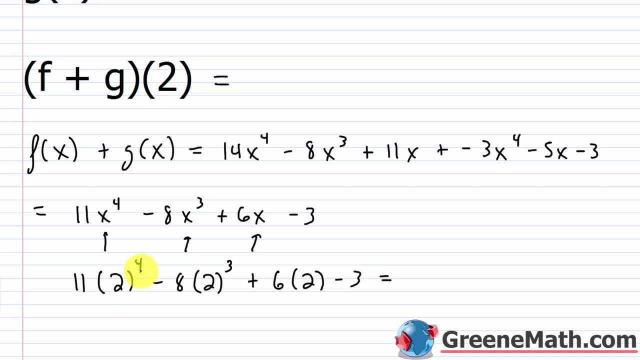 be 121.. 2 to the fourth power is 16.. 16 times 11 is 176.. We have 2 cubed, that's 8.. 8 times 8 is 64, so we're subtracting away 64.. 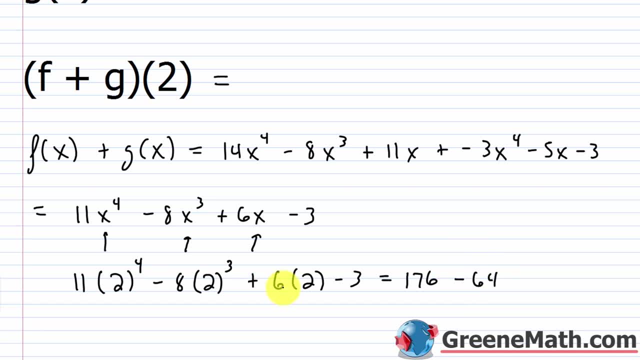 Then we're adding: 6 times 4 is 64.. So we're subtracting away 64.. Then we're adding: 6 times 2 is 12.. Then we're subtracting 3.. So 176 minus 64 is 112.. If I then add 12, I get 124. 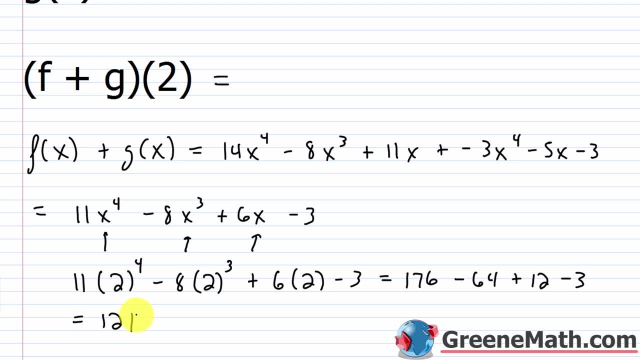 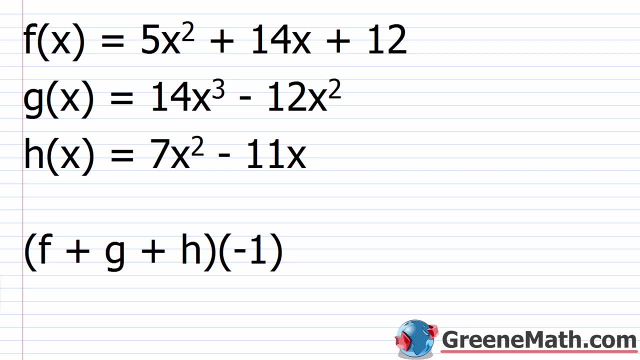 If I subtract 3, I get 121.. So again, f plus g of 2 is 121.. All right, so let's take things up just a notch. So suppose you had f of x equals 5x squared plus 14x plus 12, and g of x equals. 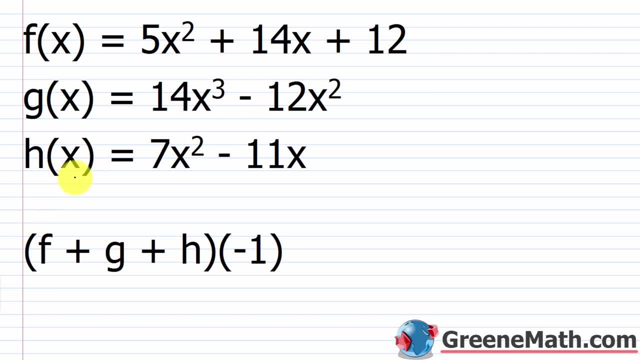 14x cubed minus 12x squared, And then h of x. the third function is equal to 7x squared minus 11x. If we wanted to find f plus g plus h of negative 1, what would we do? Well, one thing we could do is we could find f of x. 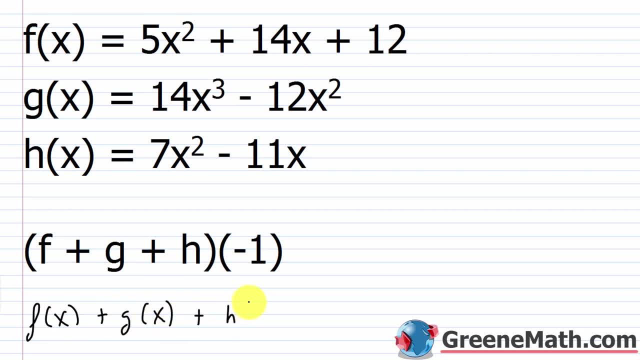 plus g of x plus h of x first, and then we could take that result and we could plug in a negative 1 for x. So let's just go ahead and crank this out. So we would have: f of x is 5x squared. 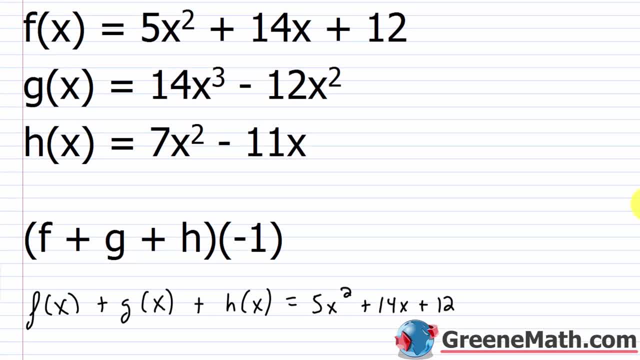 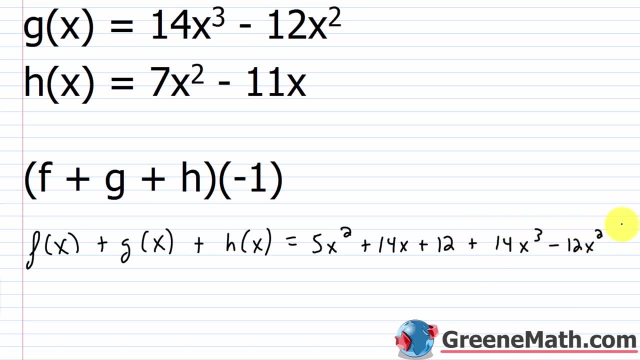 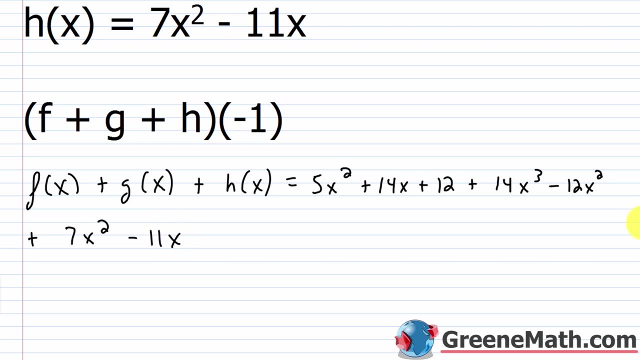 Plus 14x plus 12.. And let me scroll down: Plus g of x, which is 14x cubed minus 12x squared, Plus h of x, which is 7x squared minus 11x. Again, once I have this notation. 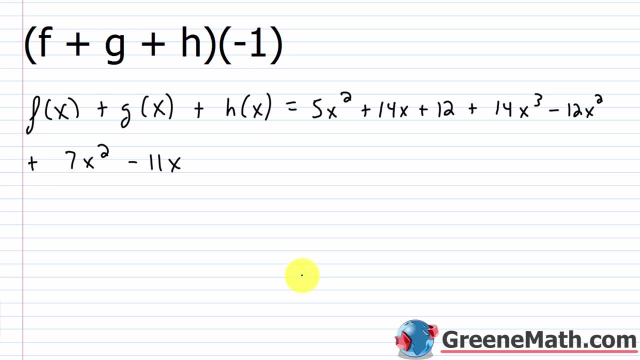 down. it's pretty easy, because all I'm really doing is just adding polynomials. So my highest exponent is a 3.. So let's start with 14x cubed, nothing to combine with that, I've got 5x squared, I've got negative 12x squared and I've got 7x squared. Well, I 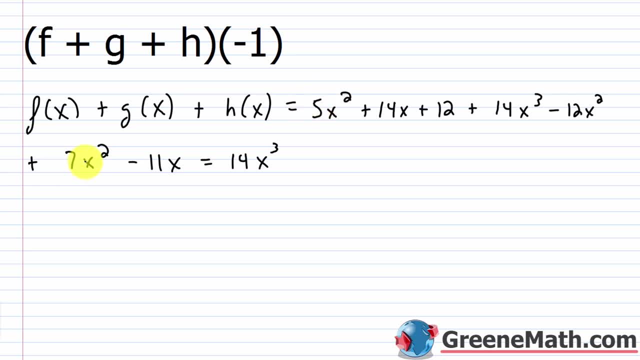 know that 5 and 7 make 12.. So 5x squared plus 7x squared would be 12x squared. Then I've got a negative 12x squared. Those would cancel out. Then I'd have 14x and negative 11x. That. 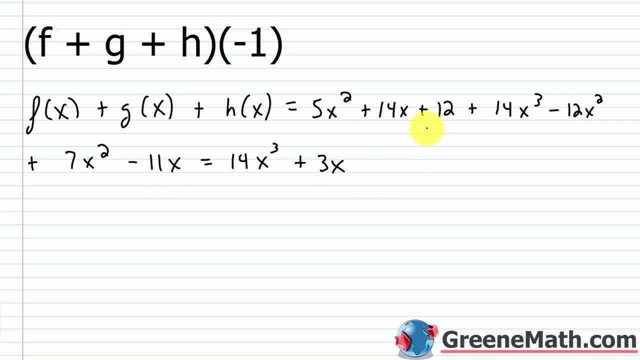 would give me positive 3x, And then, lastly, I'd have plus 12.. So what I have now is I have f plus g plus h of x, And this equals 14x cubed plus 3x plus 12.. So to find f plus g plus h of negative 1,. 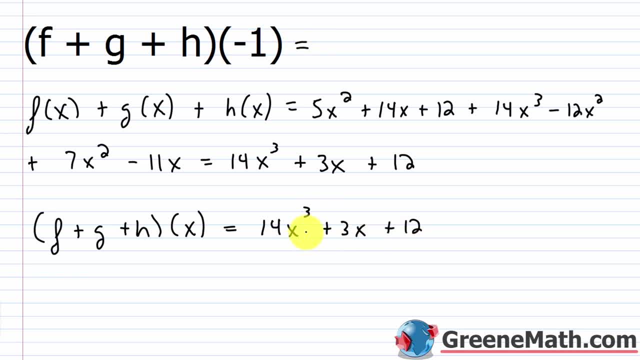 all I would do is take this and I would plug a negative 1 in everywhere I see an x, So I would have 14 times. you plug in a negative 1 for x and that's cubed, plus 3 times negative 1, plug that in for x plus 12.. Let me kind of slide this stuff down just a little bit. 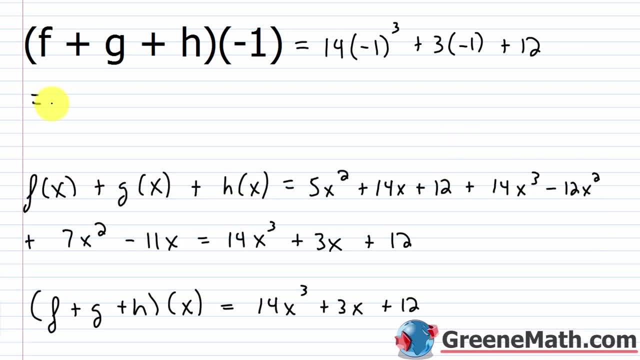 Give myself a little room. So this is equal to negative. 1 cubed is negative 1.. So negative 1 times 14 is negative 14.. 3 times negative 1 is negative 3. So we'd have minus 3.. And 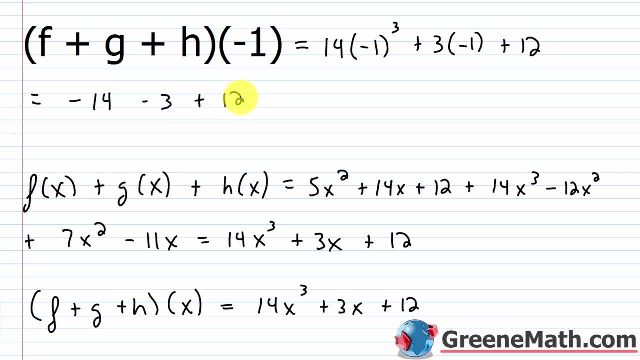 then plus 12.. So negative 14 minus 3 would be negative 17. Negative 17 plus 12 is equal to negative 5. So f plus g plus h of negative 1 is going to be negative 5.. All right, so. 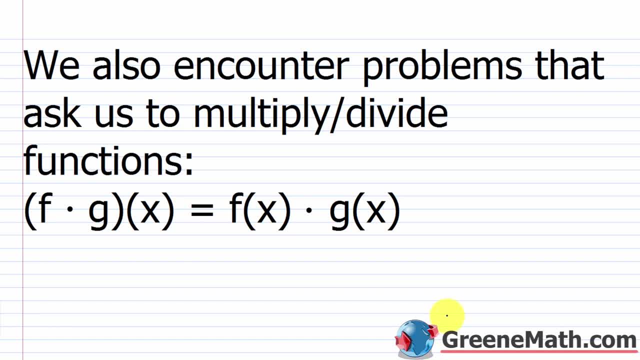 let's talk about adding and subtracting functions, Let's talk about multiplying and dividing functions, So we also encounter problems that ask us to multiply or divide functions. So if I see something like f times g of x, this is asking me for f of x times g of x Again. 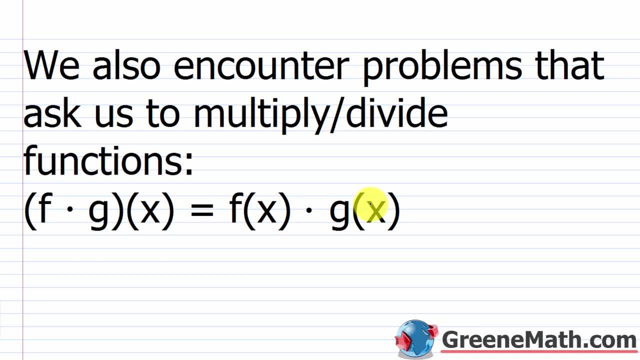 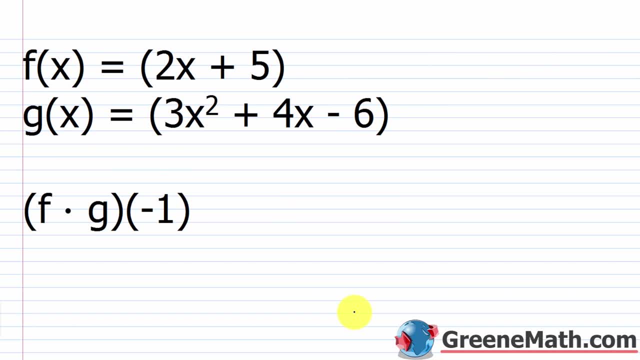 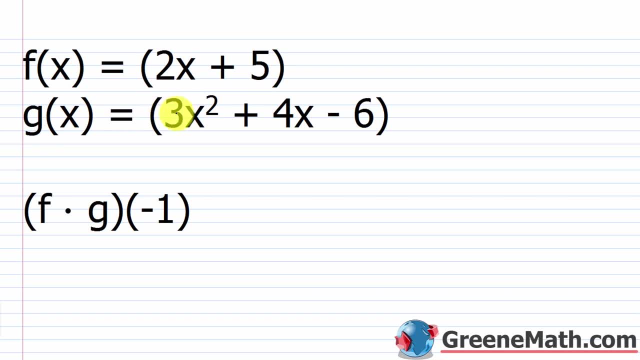 of x, which is equal to 3x squared plus 4x minus 6.. And we have f times g of negative 1.. So what this is telling me to do is multiply f of x times g of x, And I can take that result. 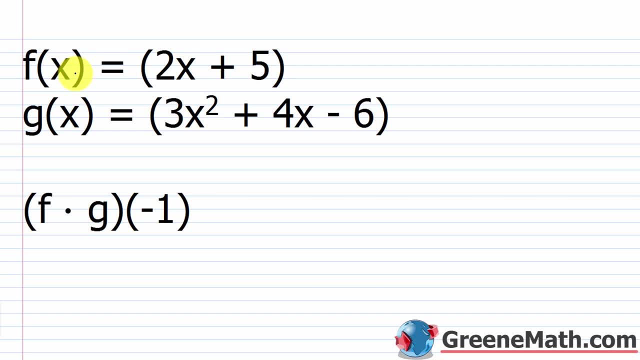 and plug in a negative 1 for x. The other thing I would do, which might be a little quicker in this scenario, is find f of negative 1. And multiply that by g of negative 1.. Either way I would get the same answer, And again. 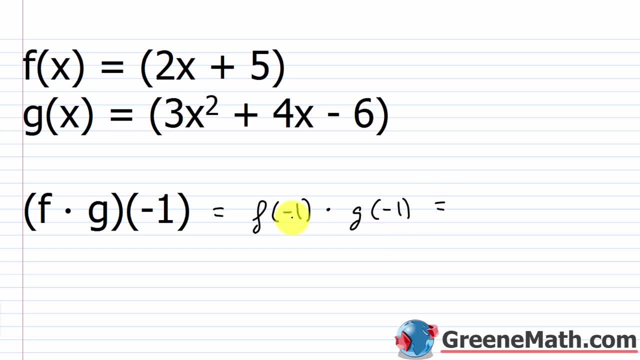 I'll show that to you. So let's start out by doing it this way. So f of negative 1. If I plug in a negative 1 for x, I'd have 2 times negative 1, which would be 1.. This 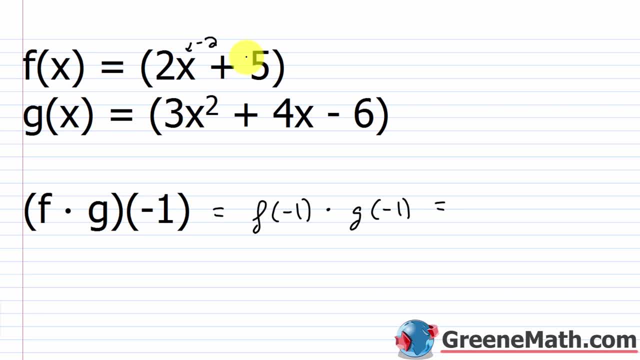 would be negative 2.. Negative 2 would then be added to 5. That would give me 3.. So you'd basically have 3 here times. If I plug in a negative 1 here, Negative 1 squared is 1.. So I'd have 1 times 3, or 3.. 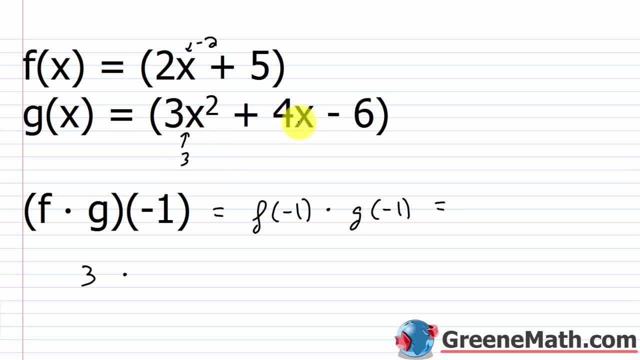 So this is 3.. I'd have 4 times negative 1, which is negative 4. So this is negative 4. And this is minus 6.. So 3 minus 4 is negative 1. And then negative 1 minus 6 is negative. 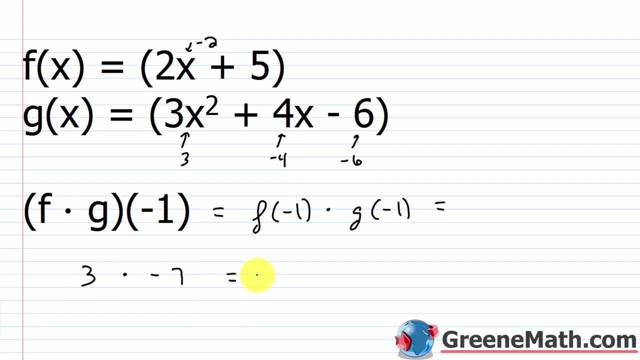 7. So this ends up being 3 times negative 7, which is negative 21.. Now that went by very, very quickly because of the way I did it. If we did it the other way, We're going to take a little bit longer, for the simple fact that I've got to multiply. 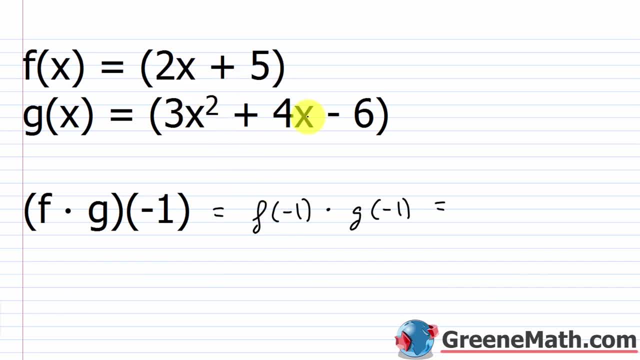 these two polynomials together first, And that can be quite tedious sometimes, So let's do it the other way. So let's say that we said that we wanted to do f of x times g of x. What would that be equal to? Well, we would have 2x plus 5 multiplied by. We have that. 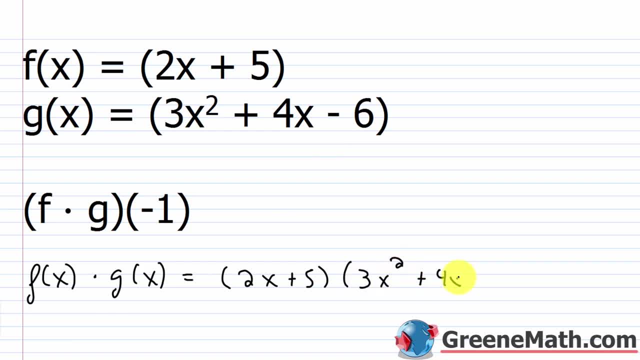 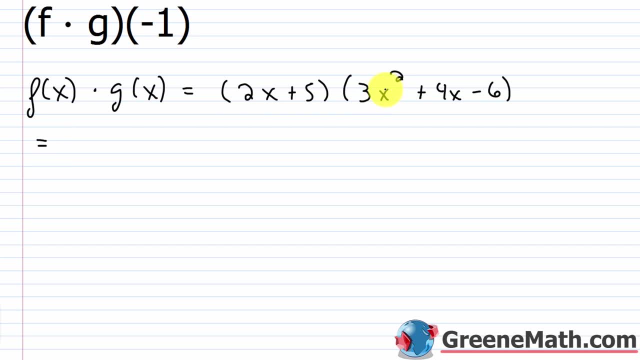 other polynomial, 3x squared Plus 4x minus 6.. So let's go ahead and crank this out. So let me take 2x and multiply it by 3x squared. That would give me 6x cubed. 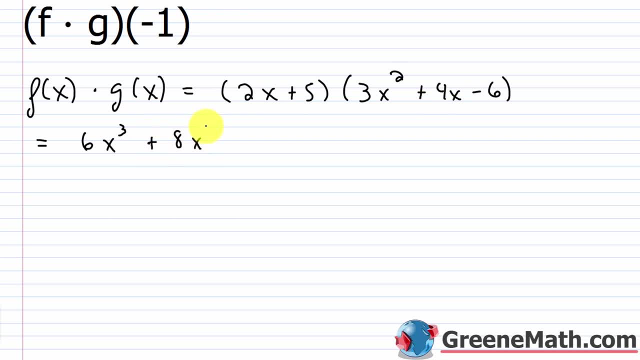 Then 2x times 4x would give me Positive 8x squared. Then 2x times negative, 6 would be minus 12x. Now I have 5 times 3x squared, That is plus 15x squared. 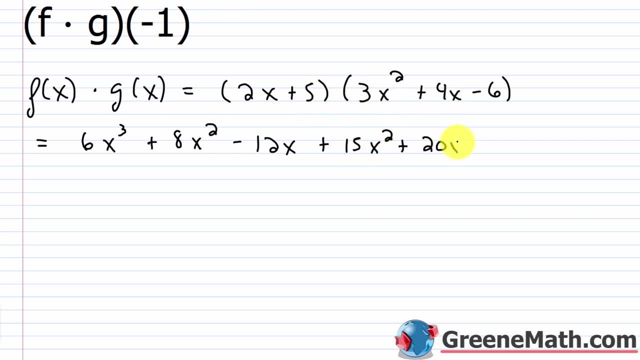 I have 5 times 4x, That is, plus 20x. Next, five times negative six, which is minus 30.. All right, So looking at this now I just need to combine like terms. So I have my 6x cubed, okay, my 6x cubed. Nothing to combine with that Then. 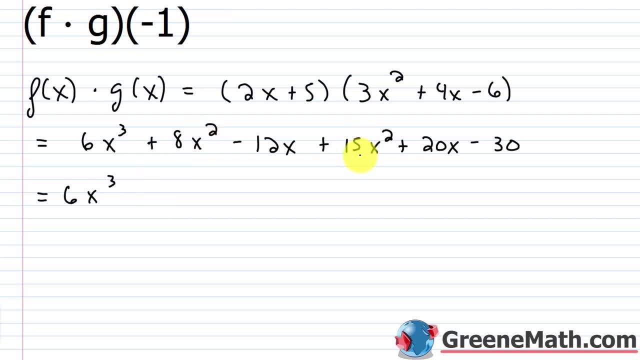 I have 8x squared and 15x squared, So what that would give me is 23,. okay, positive 23x squared. Then next I have negative 12x plus 20x. That's going to give me 8x. okay, so plus 8x. 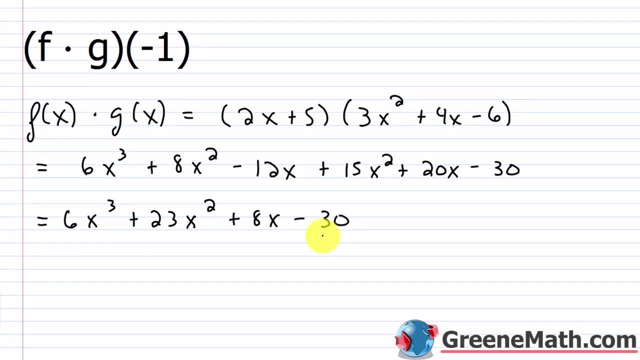 And lastly, I have minus 30. So then, once we have it in this format, I would just plug in a negative 1 for x. So f times g of negative 1 would be 6 times plug in a negative 1 for x. that's cubed. 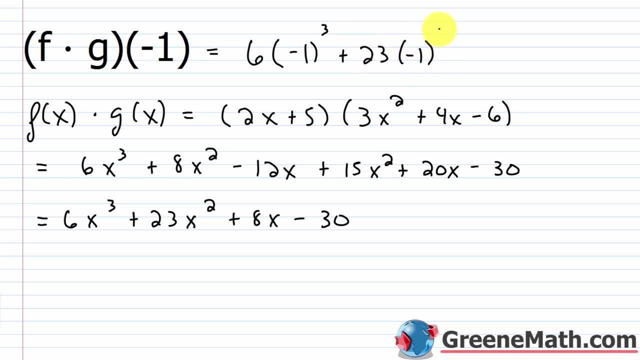 plus 23 times. plug in a negative 1 for x. that's squared plus 8 times. plug in a negative 1 for x and then minus 30. So let's scooch this down, Kind of get a little room going. So we know that. 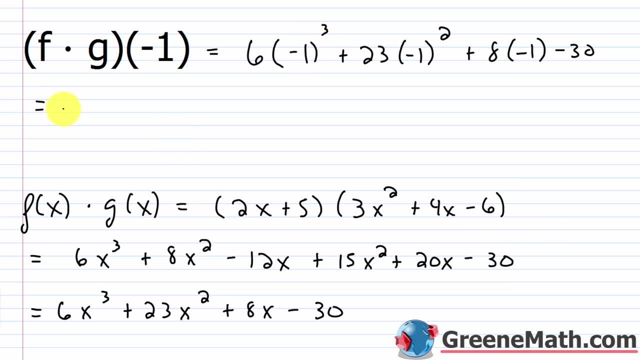 negative 1 cubed is negative 1.. 6 times negative 1 is negative 6.. I know that negative 1 squared is 1.. 23 times 1 is 23. So plus 23.. 8 times negative 1 is negative 8 and then minus 30.. So negative 6. 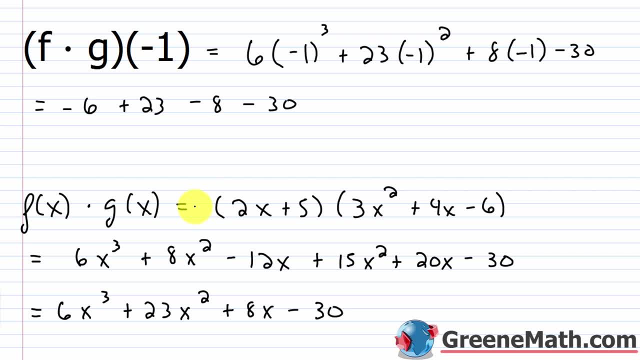 plus 23 is going to be 17.. 17 minus 8 is 9.. 9 minus 30 is negative 21.. And look how much longer it took to do it this way. When you're working with multiplication or division, it's generally. 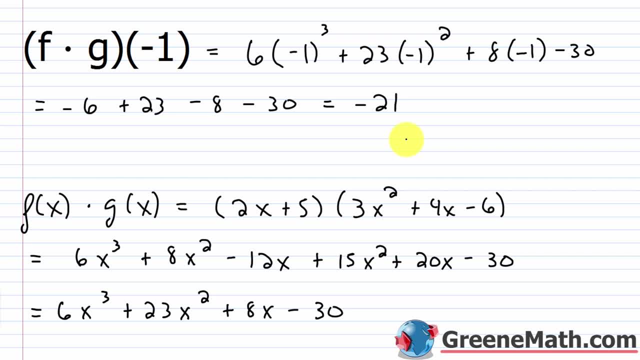 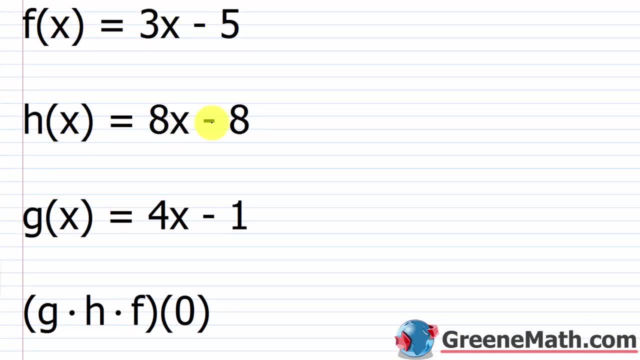 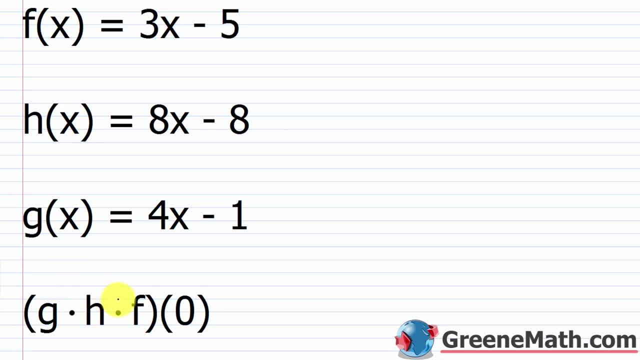 And we're asked to find g times h, times f of 0.. Again, I can do this the long way And I could say 3x minus 5 times 8x minus 8 times 4x minus 1.. And then, once I get that result, I could plug. 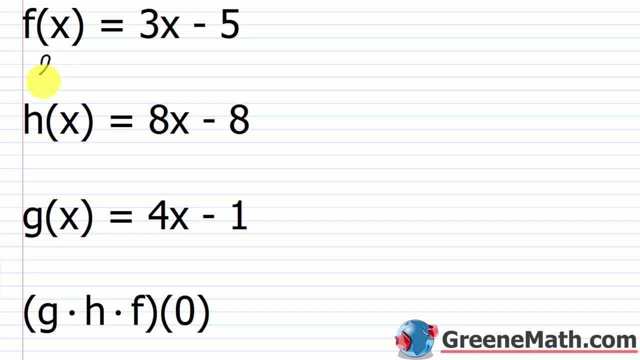 in a 0 for x. Or I could do it very quickly by finding f of 0,, h of 0, and g of 0, and then just multiplying those together. So f of 0 would be what Plug in a 0 there I'd have. 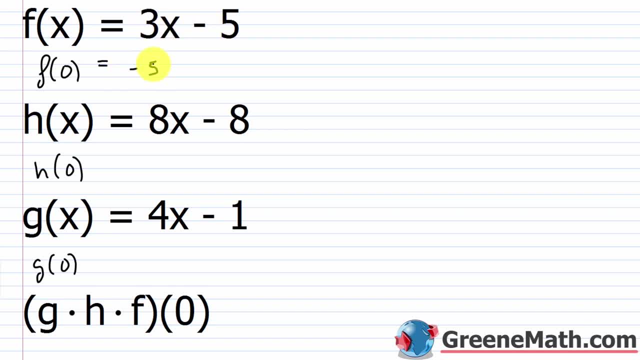 3 times 0,, which is 0, minus 5.. So this would be negative. 5.. h of 0,: 8 times 0 is 0. You'd have minus 8 or negative. 8. g of 0,: you'd have 4 times 0,, which is 0, then minus 1.. So this is equal to. 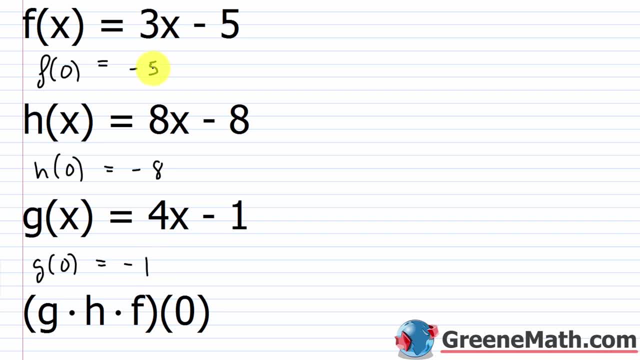 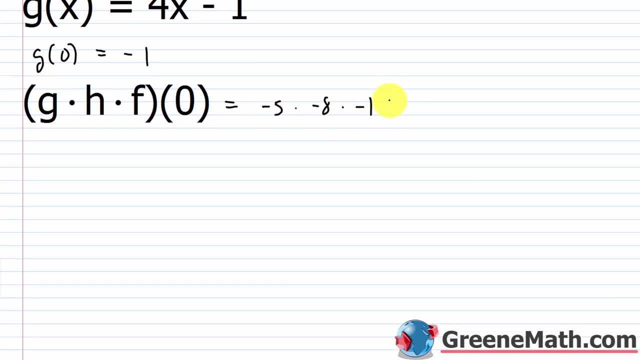 negative 1.. So, basically, what you have is negative 5, negative 5 times negative, 8 times negative 1.. And what's that going to give me? Well, if I do negative 5 times negative 1, I get 5.. 5 times negative 8 is negative 40.. All right, So let's take a look at one more, And this one's 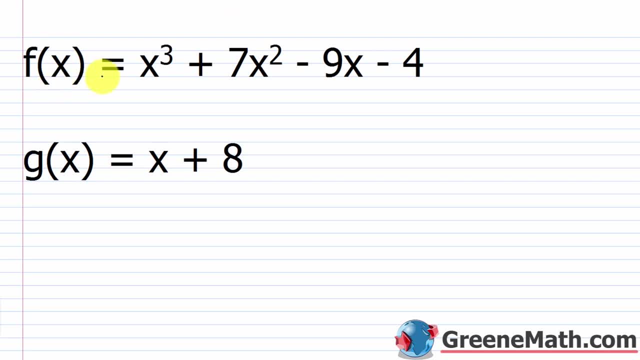 going to involve division. So let's suppose I have: f of x is equal to x cubed plus 7x squared, minus 9x minus 4.. And then g of x is equal to x plus 8.. So what I'm asked for and I'm going to 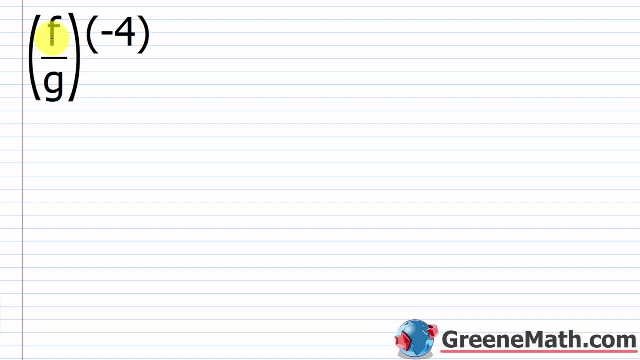 show you this. on the next page I'm asked to find f over g of negative 4.. So what this is saying is: I want f of x over or divided by g of x. When I get the result, I want to plug in a negative 4 for x. So again you can do this. the 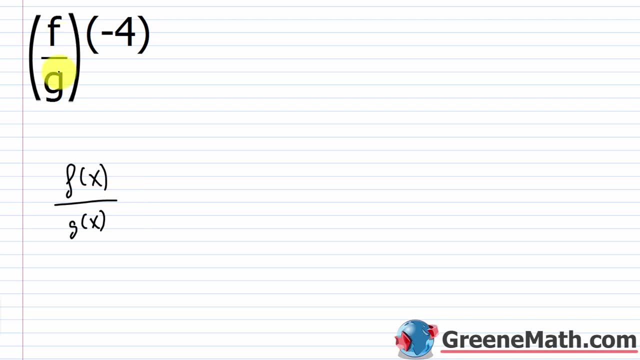 fast way: Plug in a negative 4 for x in each function and then do the division, Or the slow way which would be to crank out f of x over g of x and then plug in a negative 4.. So let's do it. 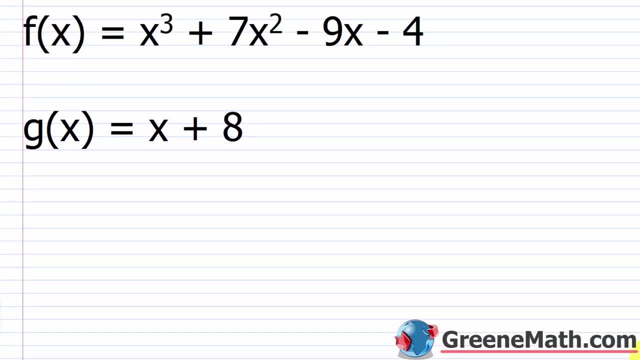 each way, And I'm going to start out with the quick way. So if I plug in a negative 4, in other words, if I had f of negative 4 here and if I had g of negative 4 here, what would I have? Well, 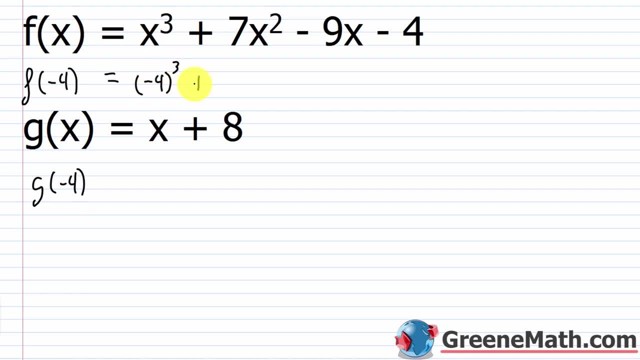 this would be: negative 4 cubed plus 7 times negative 4 squared minus 9 times negative 4 minus 4.. Negative 4 cubed would be negative 64. So that's negative 64.. Negative 4 squared would be: 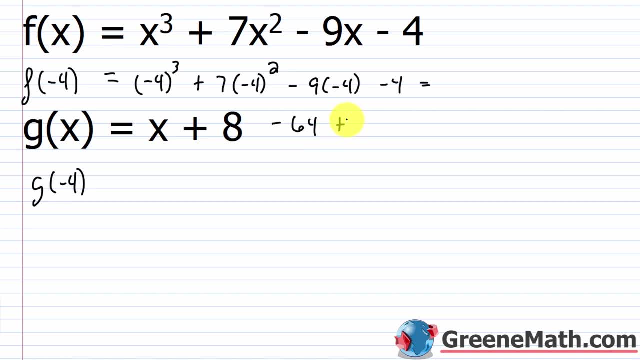 16.. 16 times 7 is 112. So plus 112.. Negative: 9 times negative: 4 is positive 36, and then minus 4.. Negative: 64 plus 112 is 48.. 48 plus 36 is 84. And then 84 minus 4 is 80. So I could say f of negative. 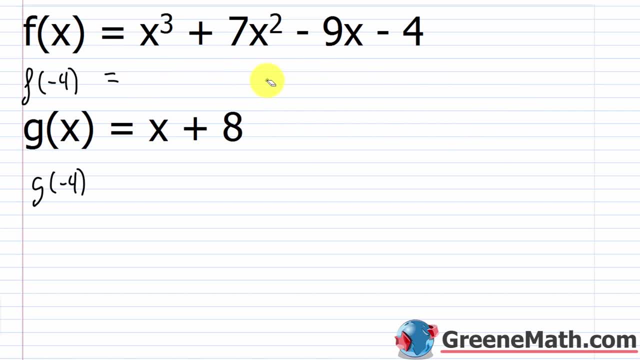 4 is 80.. So what's g of negative 4?? If I just plug in a negative 4 there, I'm going to get a negative 4.. I know that negative 4 plus 8 would be 4.. So now all I want to do, if I want f over g. 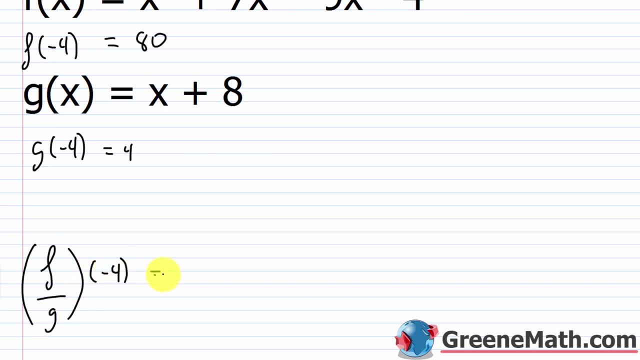 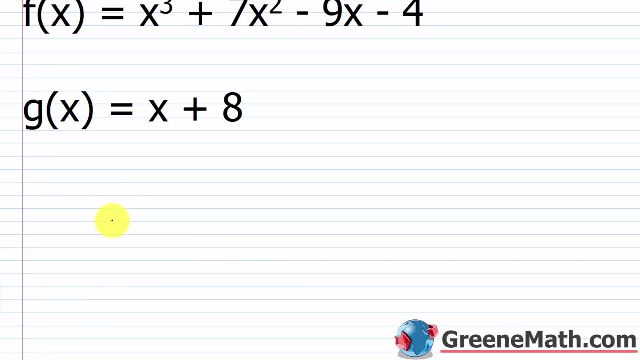 of negative 4,. I know it's 80 divided by 4, which is just 20.. Okay, so that's my answer. To kind of do this the long way, I would take f of x and divide it by g of x And again. 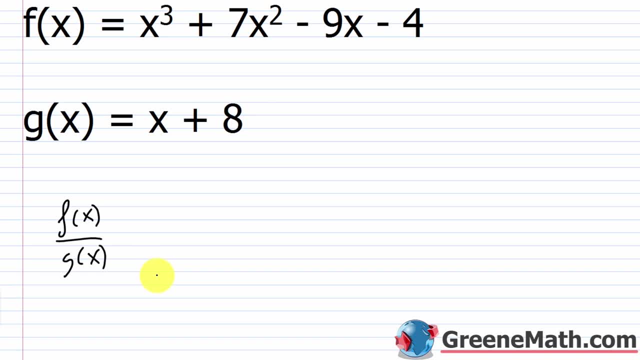 when I'm done with that, I would plug in a negative 4 for x, And again you'd find out that the value you get is 20.. So I'm going to plug in a negative 4 for x, And again you'd find out. 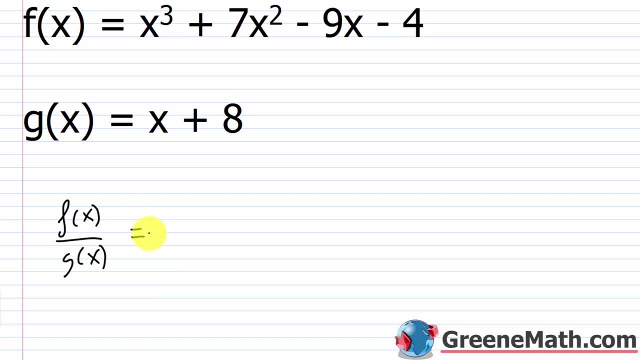 that the value you get is 20.. So let's go ahead and do this the long way. So I would have x cubed plus 7x squared minus 9x minus 4 over x plus 8.. Now what's the quick way to do this? 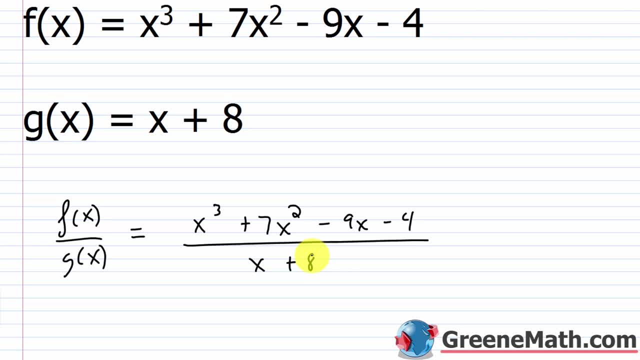 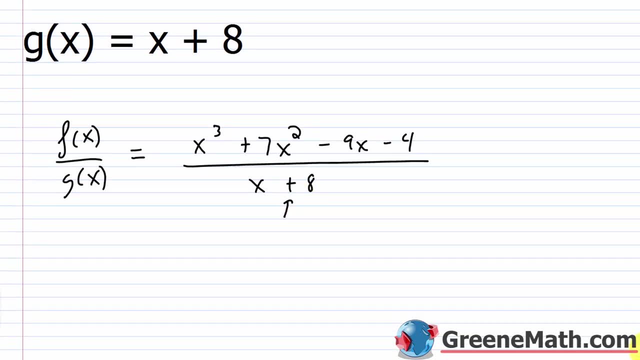 We just, in the last lesson, learned about synthetic division And we see that we have a perfect scenario for synthetic division And all I need to do really is convert this x plus 8 into x minus 7x squared. So I'm going to plug in a negative 4 for x plus 8.. And again you'd find: that the value you get is 20.. So let's go ahead and do this the long way. So I would have x cubed plus 7x squared minus 9x minus 4 over x plus 8.. Now what's the quick way to do this? We just, in the last lesson, learned about synthetic division, And again you'd find that the value you get is 20.. So let's go ahead and do this the long way. So I would have x cubed plus 7x squared, minus 9x plus 8.. Now what's the quick way to do this? 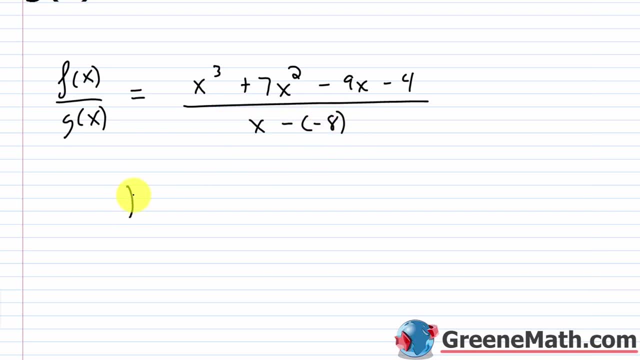 a negative 8.. So I could divide this very quickly with synthetic division. I'll use my coefficients here: 1,, 7,, negative 9, and my constant negative 4.. And I'm going to use my value negative 8 out here. put my little line there, drop this 1 down and I'll get going. 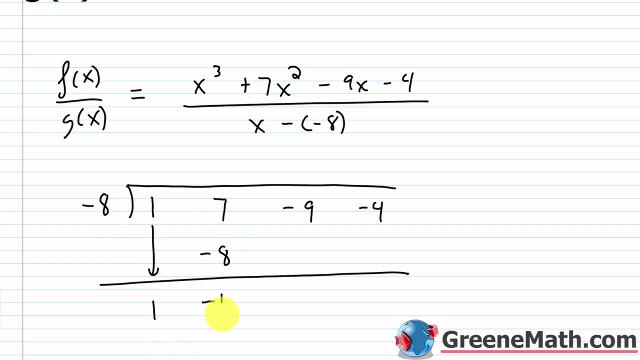 Negative 8 times 1 is negative 8.. 7 plus negative 8 is negative 1.. Negative 8 times negative: 1 is positive 8.. Negative 9 plus 8 is negative 8. And I'm going to use my value negative 8 out here. 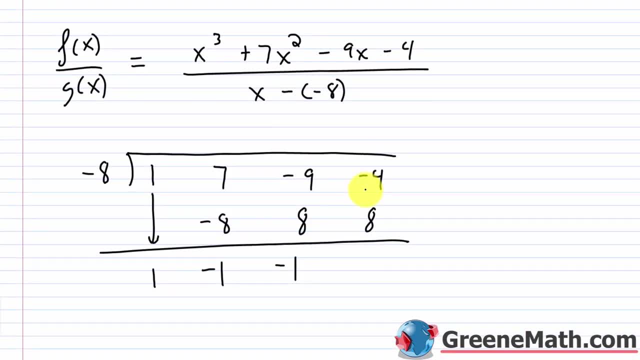 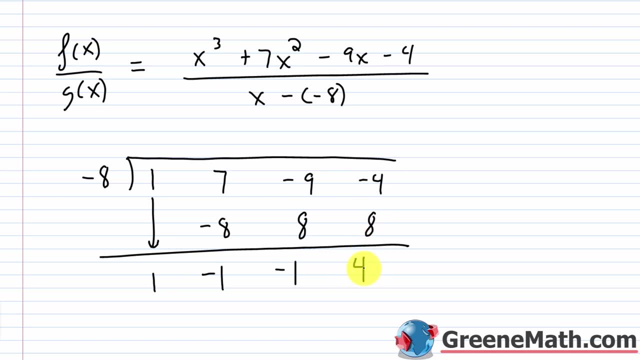 negative 1.. Negative 8 times negative 1 is 8.. Then I would want to do negative 4 plus 8. That would give me positive 4.. So I already have my answer now. Remember: the degree of this polynomial in the answer is one less than the degree of the polynomial here, Since this is x. 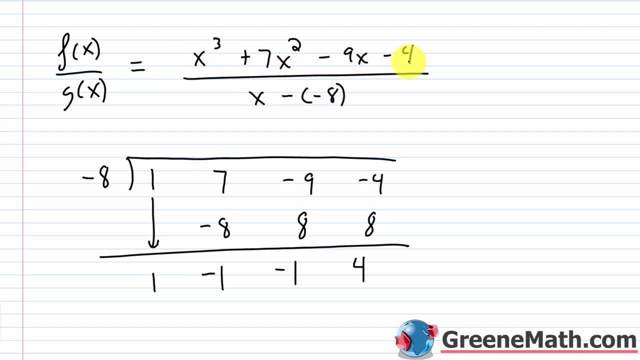 cubed as the highest power. this polynomial has a degree of 3.. The highest exponent is a 3.. Here, the highest exponent would be a 2. It's of degree 2.. So this would be the coefficient for x squared. This would be the coefficient for x to the first power. This would be your. 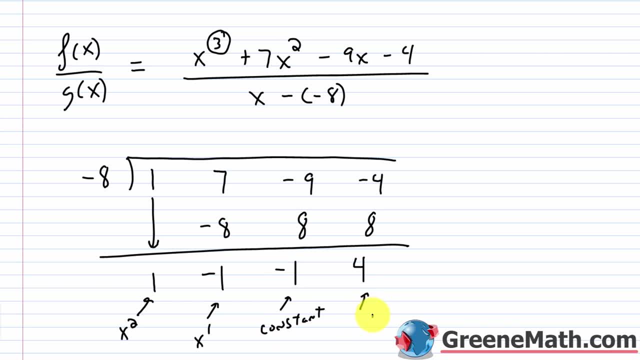 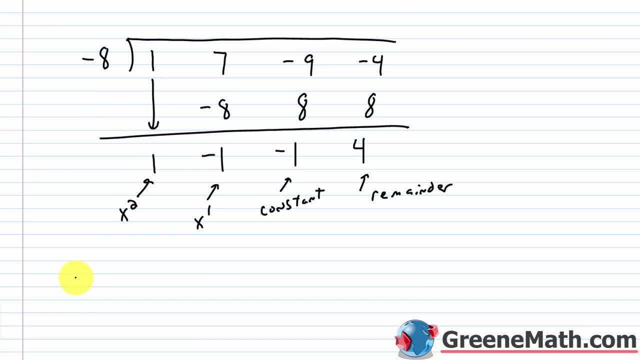 constant And this would be your remainder. Okay, All right. So if we wanted to write this, you would have 1x squared, or just x squared minus 1x to the first power, or just minus x and then minus 1 and then plus 4 over. Your divisor was x plus 8.. 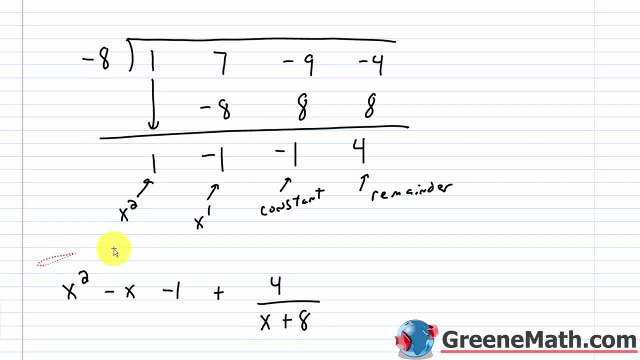 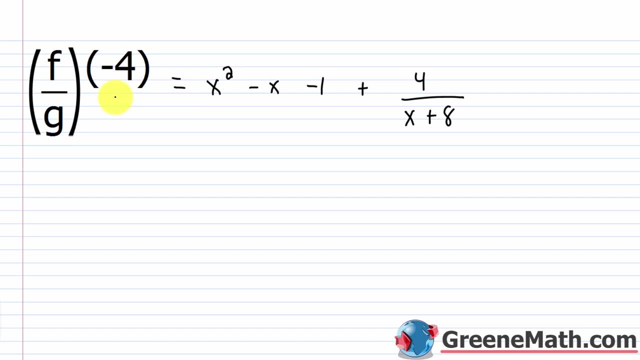 x plus 8.. So let's copy this. It will come down here. We'll put: this is equal to this: f over g of negative 4 is equal to this: if we substitute in a negative 4, everywhere we see an x. 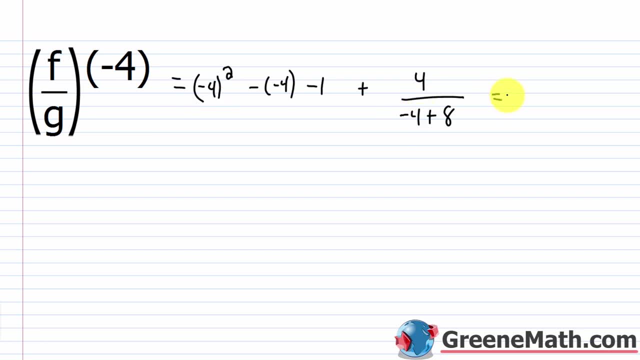 Okay. So if I had negative 4 squared to begin, negative 4 squared is 16.. Then, minus a negative 4 is the same thing. So I'm going to write this, I'm going to write this, I'm going to write this. 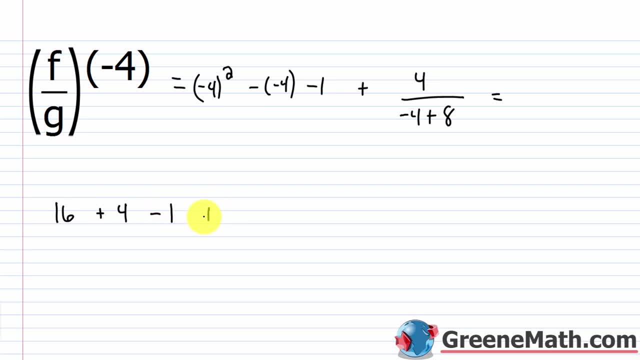 Same thing as plus 4. Then you'd have minus 1. Then plus Here you have 4 over, You have negative 4 plus 8. Negative 4 plus 8 is 4.. 4 over 4 is 1. So essentially you can see that these two would. 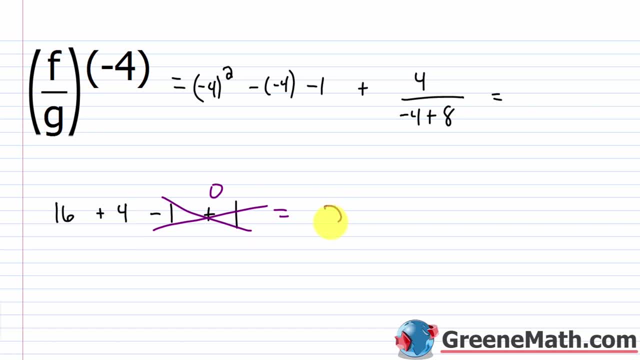 cancel at 0. You're left with 16 plus 4, which is 20.. And again, that's what we got at the very beginning of this: very easily, just by plugging in a negative 4 for x in each function and dividing. 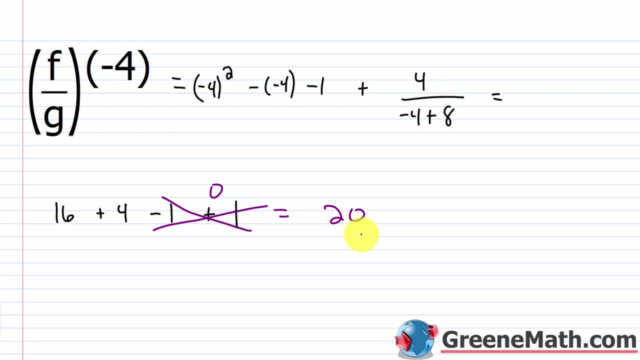 right, You had 80 divided by 4, which gave you 20 as well. So much, much quicker to do it that way, But I wanted to go through it the long way just to prove to you that it works either way. 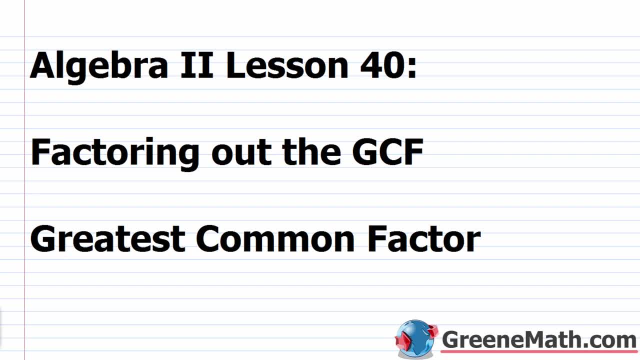 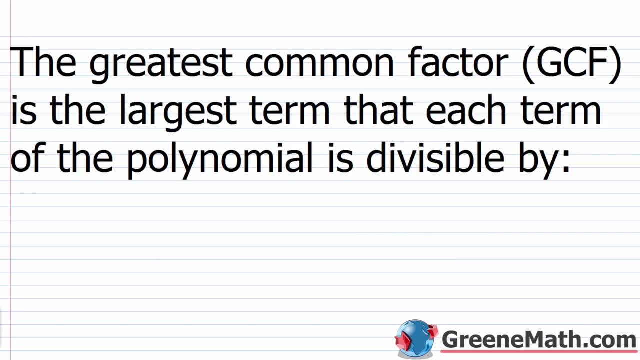 Hello and welcome to algebra 2, lesson 40. In this video, we're going to learn about factoring out the GCF, otherwise known as the greatest common factor. Now, before we actually get into factoring, I need to review something known as the greatest common factor, or the GCF. This is how we abbreviate. 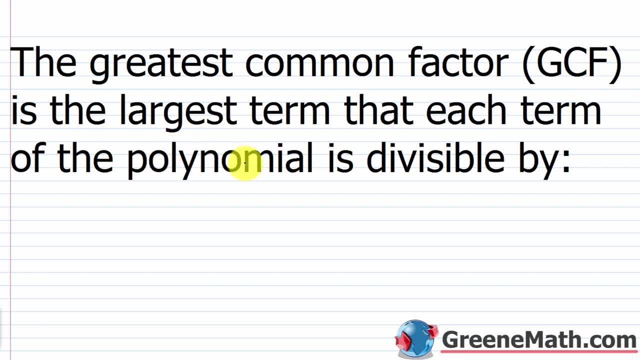 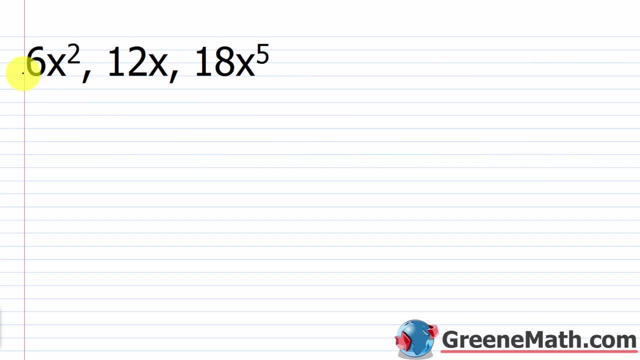 So this is the largest term that each term of the polynomial is divisible by. So I want to start out with a brief example. So we want to find the GCF for 6x squared 12x, and then 18x to the fifth. 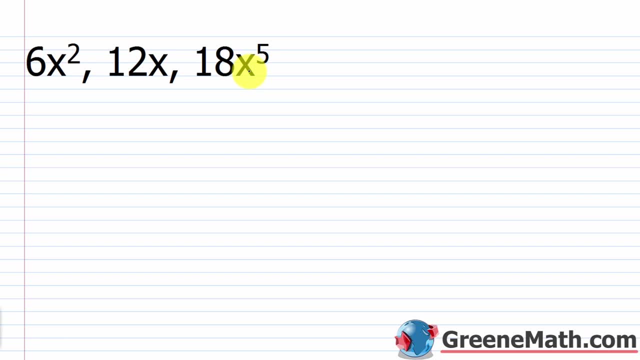 column. So for the number part, we've been doing this since pre-algebra. okay, If I wanted to find the GCF for 6,, 12, and 18,, a lot of you at this point can eyeball that and say, well, I know it's. 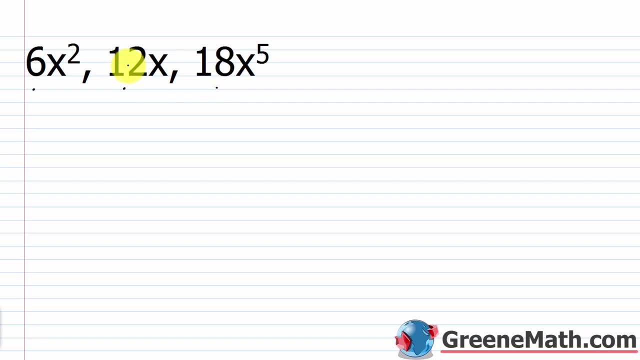 6, right, Because 18 divided by 6 is 6.. So I'm going to find the GCF for 6x squared 12x to the sixth would be 3,. 12 divided by 6 would be 2,. 6 divided by 6 would be 1, right, So that's easy to. 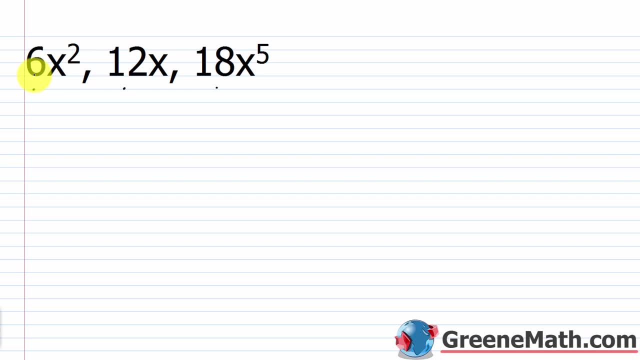 do at this point for us. but if you have no clue on how to do it, the official procedure would be: you take each number and you find the prime factorization. So 6 would factor into 2 times 3.. 2 is prime, and so is 3.. 12 we could factor as 4 times 3.. 3 is prime, 4 is going to be 2 times 2,. 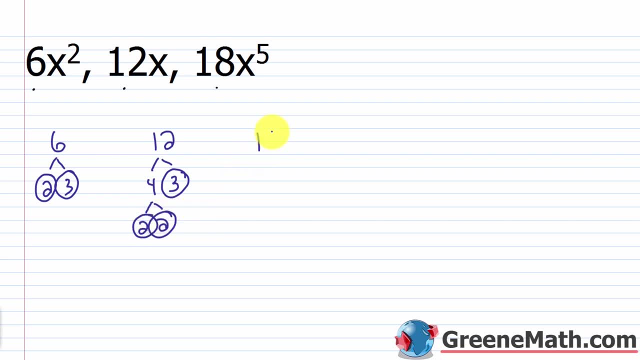 and 2 is prime. Next we have 18.. So 18 I could write as 9 times 2.. 2 is prime, Then 9 is 3 times 3. 3 is prime. Now, once we have the prime factorization for each number, what we're looking to see is: 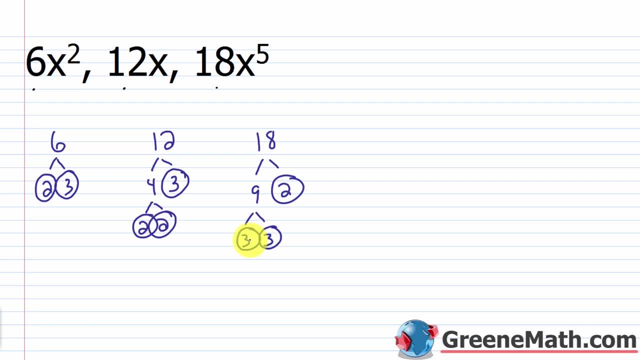 what prime factors are common to everything? okay, Common to everything. So to make that crystal clear, I could write 6 right here as 2 times- I'm going to put a big space out here- times 3.. I could write 12,. 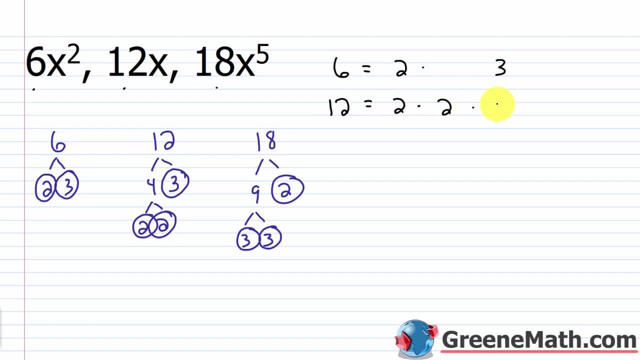 as 2 times 2 times 3.. And then I could write 18 as 2 times. leave my space 3 times 3.. Now the way I've written it here makes it easy to see what's common to everything. 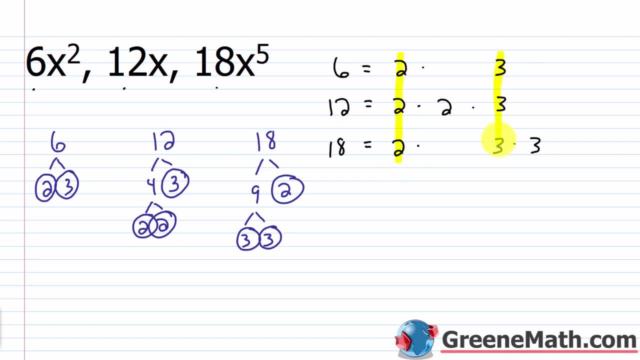 Everything has one factor of 2.. Everything has one factor of 3.. So to get my GCF for 6,, 12, and 18, I just take the prime factors that are common to everything and I multiply them together. 2 times 3 is 6,. okay, So 6 would be your GCF. And the reason for that is because 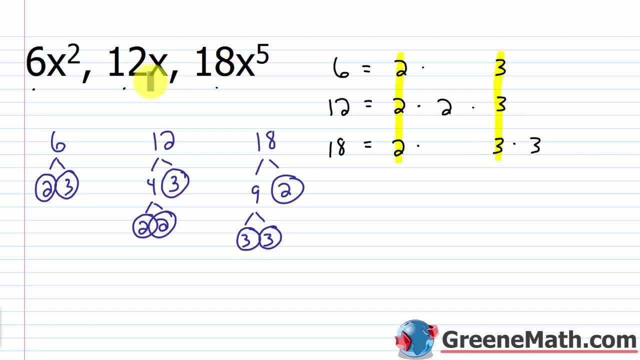 everything involved has those prime factors when the number is built. So in other words, 18 has a prime factor of 2 and a prime factor of 3.. So I know 18 would be divisible by 6.. Same thing with 12.. I know it would be divisible by 6.. And then same thing with 6.. I know it would. 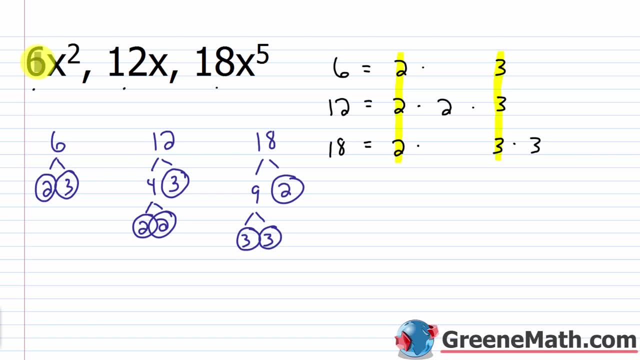 be divisible by itself: 6.. So again, the GCF is 6.. So I know it would be divisible by 6. And then let me erase all that, All right. So when we think about our GCF, I'm just going to put 6 right here. 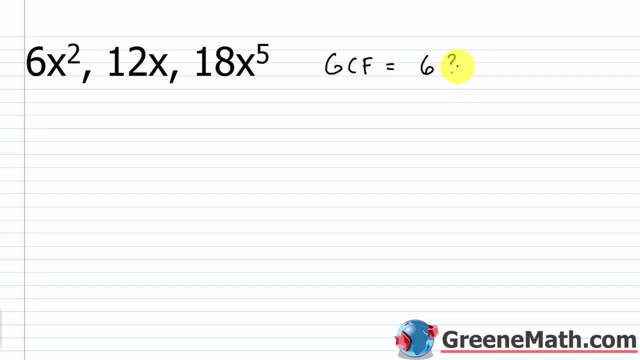 And then I'm going to put a question mark for the variable part. The variable part is pretty simple. overall, You have x squared, you have x and you have x to the fifth power. Now you could go through and do the same thing. You could factor x squared and say: 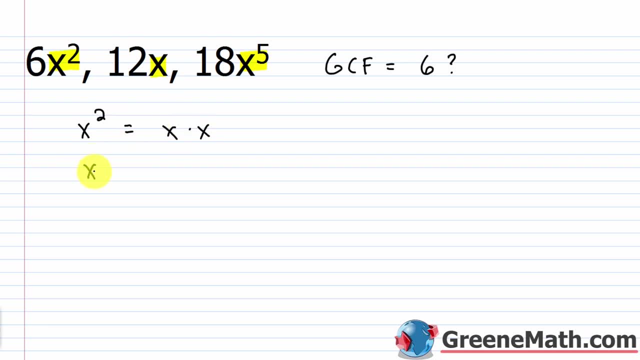 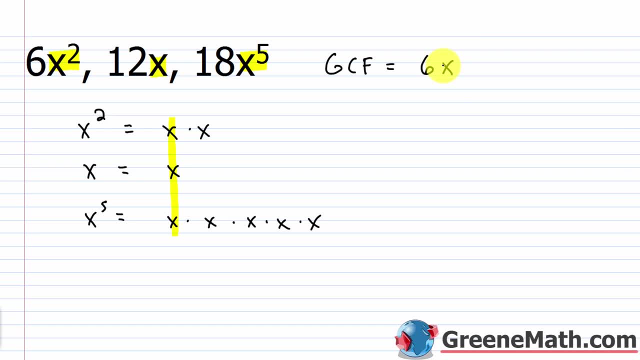 1x. But what's the quicker way to do that? Well, when you have variables involved, the first thing you want to check to make sure of is that everything has that variable. In other words, this has an x, this has an x and this has an x. 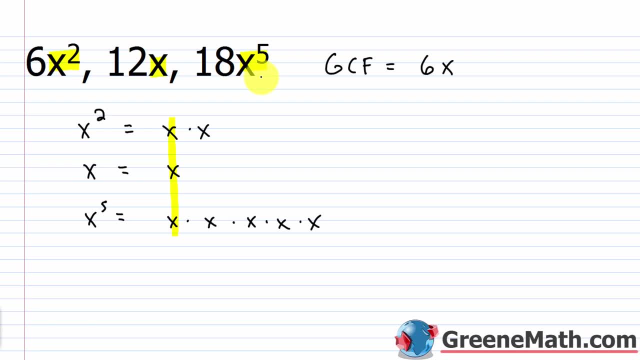 Then you're just going to look for the smallest exponent. In this case, the smallest exponent would be this one: the understood exponent of 1.. The reason you look for the smallest exponent, that's going to tell you the fewest number of factors of that variable that you're going to 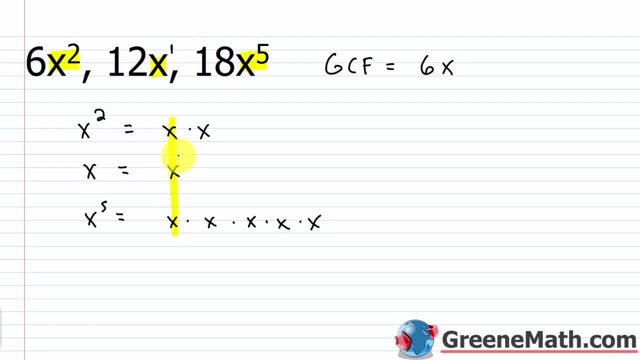 have In this case. I only have 1x here. Everything else, if this is the smallest, will have at least that, And so that's going to be common to everything. So my GCF here would be 6x. 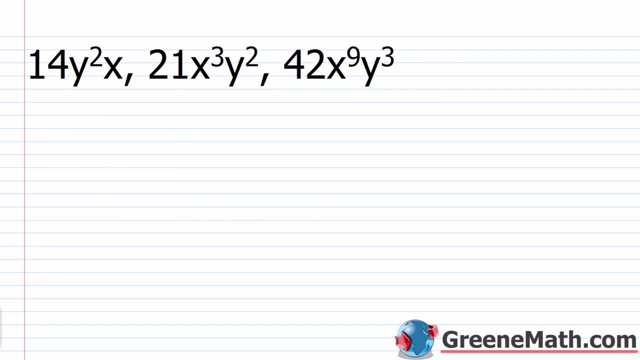 All right, let's take a look at another one. Let's say I had 14y squared x, 21x cubed y squared and 42x to the ninth y cubed. Now again, a lot of you can kind of eyeball this and look at the. 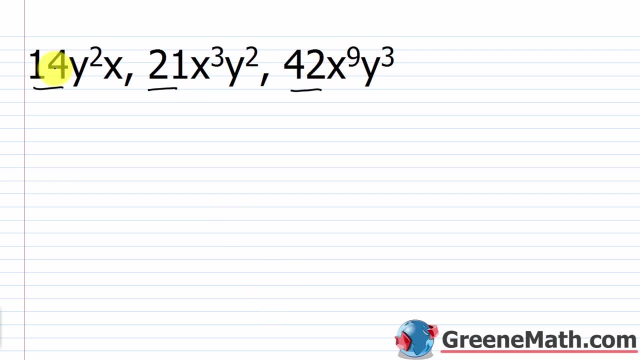 numbers and say: well, I know that 42 is divisible by 14. It would be 3.. I know that 21 is not divisible by 14, but I know that 21 and 14 would share a common factor of 7.. 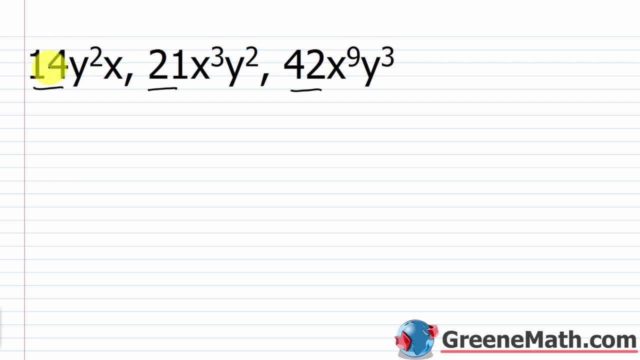 GCF, for the number part would be a 7, because 14 is divisible by 7,, 21 is divisible by 7, and 42 is divisible by 7.. So once you have enough experience you can kind of eyeball things. 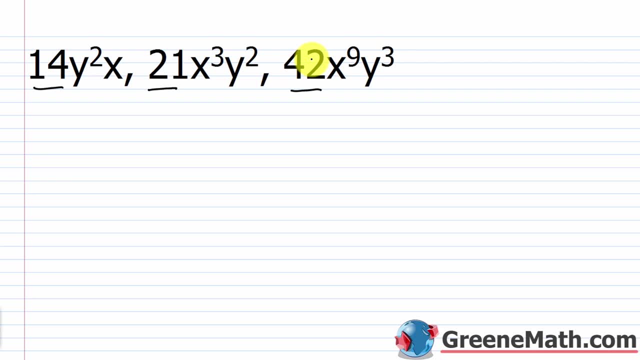 and say I know what my GCF is, But for right now I want to just go through it the long way. For those of you who are a little confused about what I just did, if I think about 14, it's what. 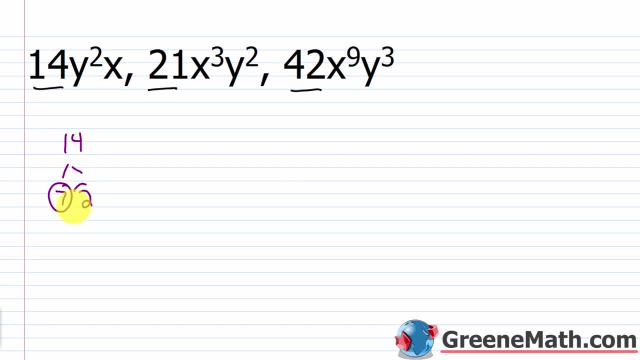 I could factor it into 7 times 2.. 7 and 2 are both prime numbers. If I think about 21,, I could factor times 3.. 7 and 3 are both prime numbers. When I think about 42, I could factor that into 7 times. 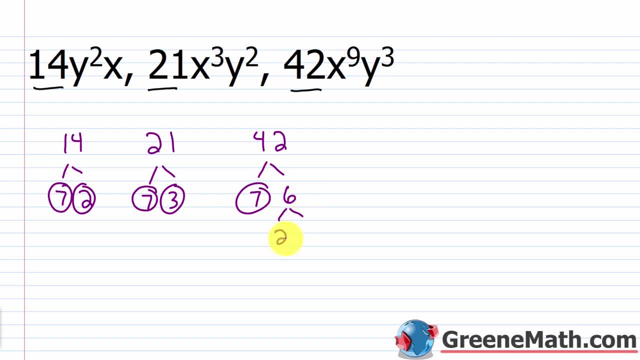 6. 7 is prime. 6. I could factor into 2 times 3.. 2 and 3 are both prime. So look at what's common to everything. Everything has one 7.. And then this does not have a 3. This does not have a 2.. 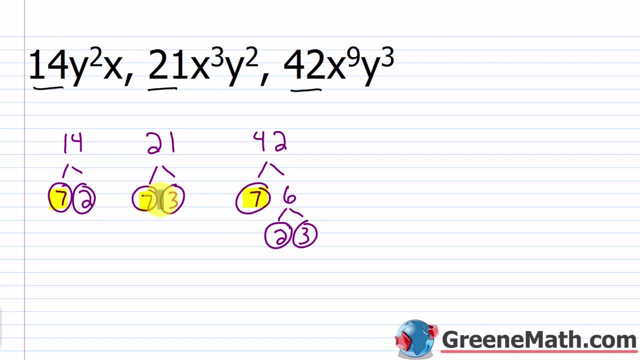 So a 2 would not be common to everything And a 3 would not be common to everything. So I can only take what's common to everything, And that's a 7. So for the number part, the GCF would be 7. And then you have some variable there. All right, So let's erase this. 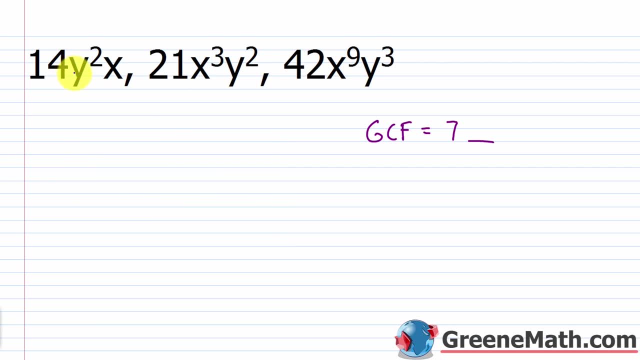 Now for the variable part. I see that I have the variable y And I have the variable x involved. Now I have an x and a y in every term here, So I'm just going to pick the smallest exponent on each. So I'm just going to write x And I'm going to write y. 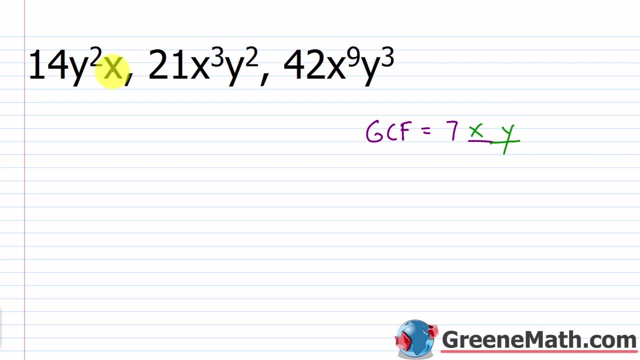 And then I'm going to write the smallest exponent that appears on each. So here for x, I have x to the first power, I have x cubed And I have x to the ninth power. So the smallest exponent is a 1.. So this just stays as x. Or you could write x to the first power like that if you. 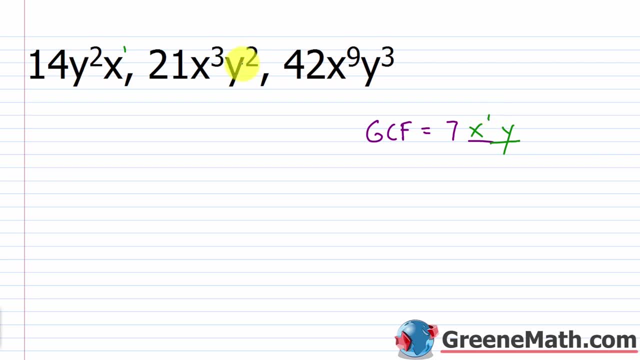 wanted to. For y, I have y squared, y squared and y cubed. The smallest exponent that appears on y is a 2. So this would be y squared here. So my GCF here is going to be 7,. 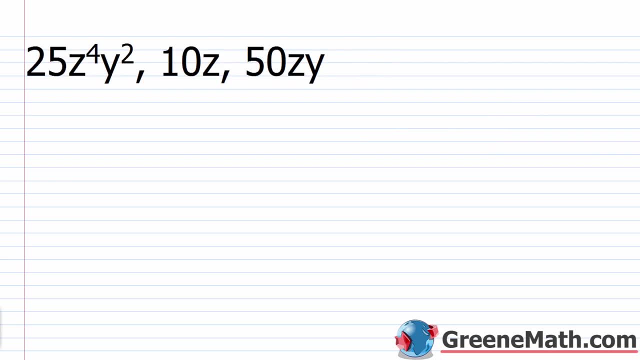 x, y squared. Well, let's do one more of these And then we'll get to some factoring. So we have 25z to the fourth power, y squared, We have 10z And we have 50zy. So for the number part again, 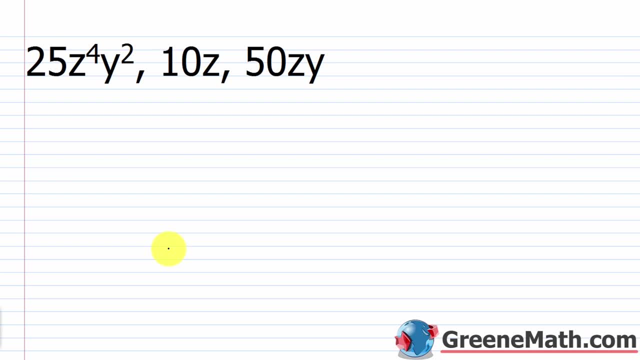 try not to get into a factor tree. Just notice that everything here is divisible by 5.. All right, We think about our divisibility rules. I know everything ends in a 5 or a 0 here. So 25 divided by 5 would be what, That would be 5.. And then we have 25z to the fourth power y squared. So we 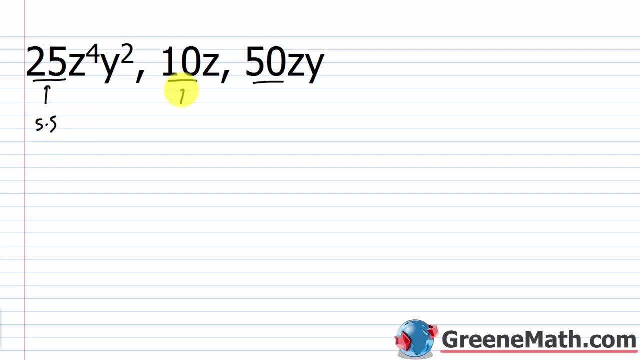 know this is 5 times 5.. 10, we know, is what? 5 times 2.. 50, we know, is 5 times 10.. Now, 10 is what It's 5 times 2.. So let me write: 5 times 5 times 2.. So I've factored each number here, But I can. 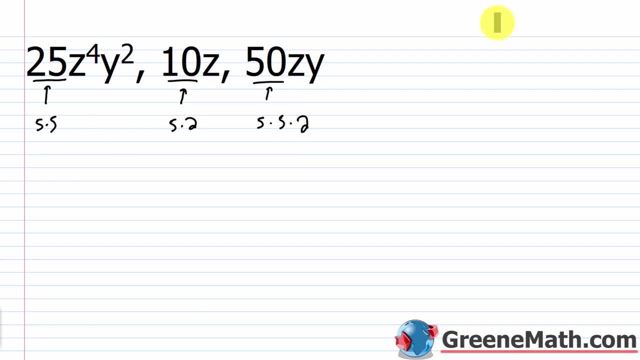 kind of do that in my head, And I know you can as well, especially with these smaller numbers. Everything has one 5.. Everything does not have a second 5. And then everything does not have a 2. So really the only prime factor that's common to everything is 5.. So for my GCF- 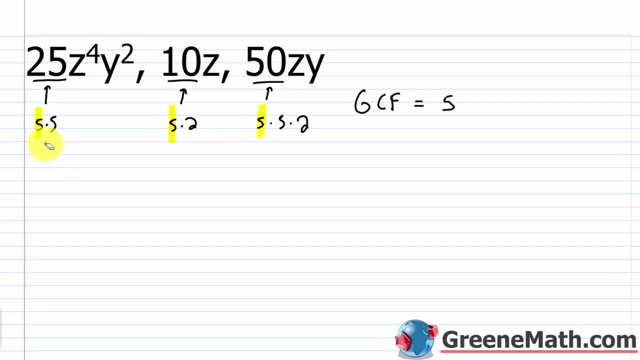 the number part would be a 5, and a 5 only. All right For the variable parts. we see we have z and we have y involved. Now I have a z here, a z here and a z here. 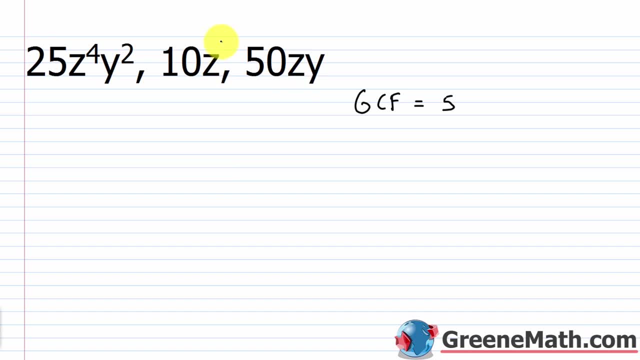 The smallest exponent that appears on z is a 1.. You have a 1 here and a 1 here, So I just put z Now for y. I have y squared here and I have y to the first power here, But I don't have a y here. 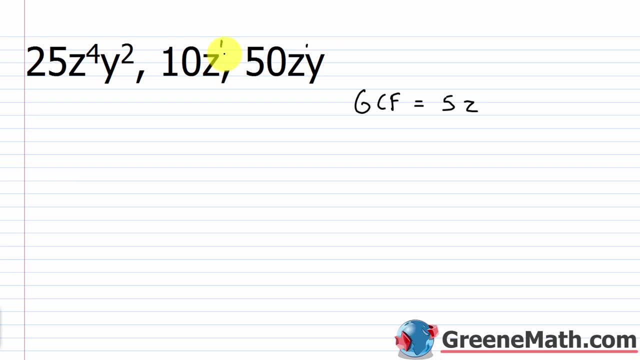 So it's not common to everything. And if it's not common to everything, it can't go into the GCF. The GCF is the largest term that each term here would be divisible by. So each term here would not be divisible by something with a y in it, because there's no y here. So the GCF is just. 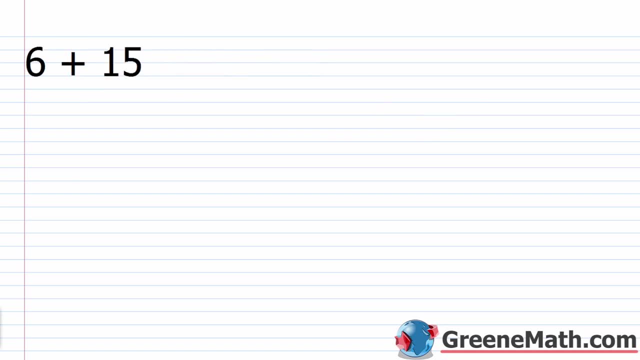 going to be 5.. So now that you know how to find the GCF for a group of terms, let's talk about how to factor out the GCF from a polynomial. To do this, I'm going to start out with a very simple example. 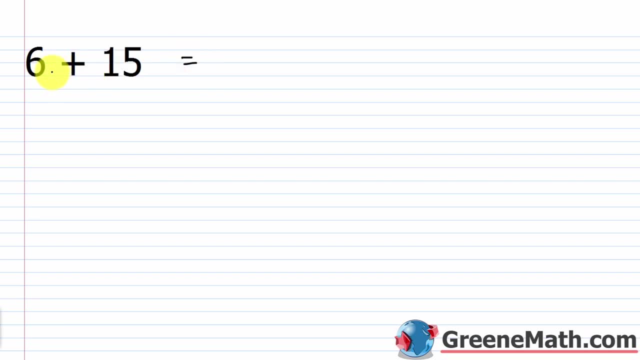 Let's say you had 6 plus 15.. And what I would do is I would write 6 as 2 times 3. And I would put plus 15, I'd write as 5 times 3.. All we're doing is we're just kind of reversing. 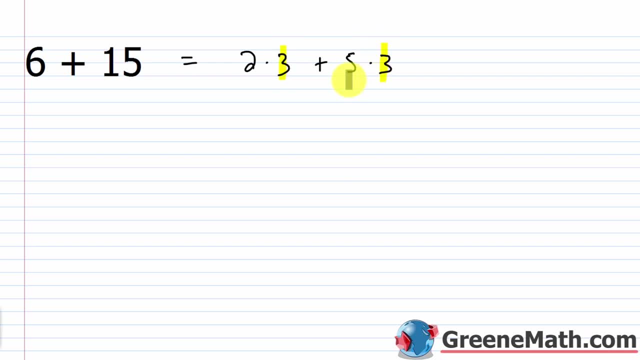 the distributive property. Notice that I have a 3 that's common to each right. 3 is the greatest common factor between 6 and 15.. All I'm going to do is pull that 3 outside of a set of parentheses, So 3 goes here And then in these spaces I'm just going to have what's left. I 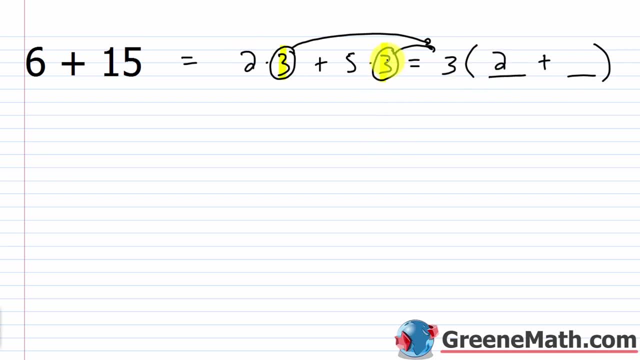 pulled out a 3 here, so I'm just going to have a 2, that's left. I pulled out a 3 here, so I'm just going to have a 5, that's left, And you can think about reversing this. If I did 3 times 2, I'd be. 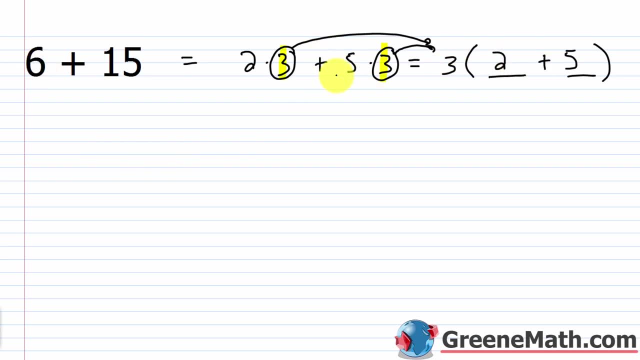 right there, right, And that would give me 6.. Then, plus, if I did 3 times 5 or 5 times 3, it's the same thing. I'd have that, which would give me 15.. So, instead of kind of going this way, like I'm normally doing, I'm just kind of going. 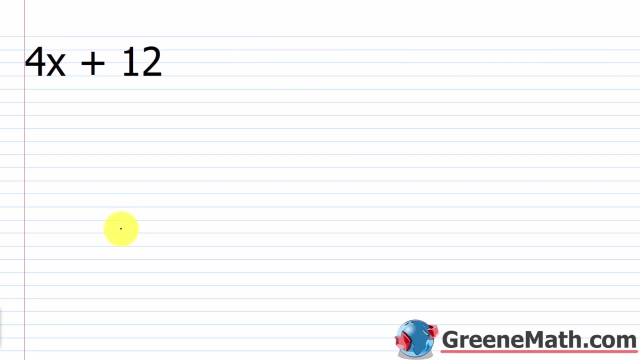 backwards. right, I'm reversing the distributive property. All right, so let's look at the first example. So we have 4x plus 12.. The first thing I'd want to do is figure out what is the GCF here. 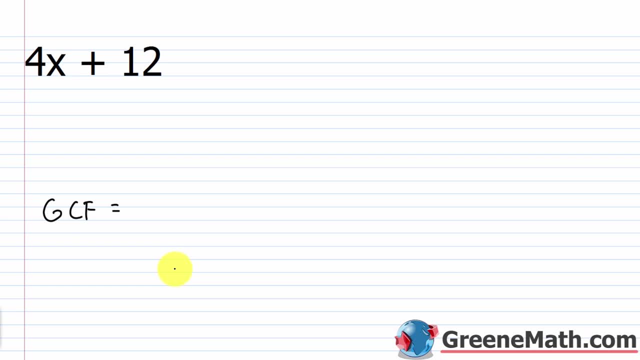 What is the greatest common factor? Well, I know there's going to be no variable involved, because I have an x here But no x here. Remember, it's got to be common to everything. So I'm just looking at a number. 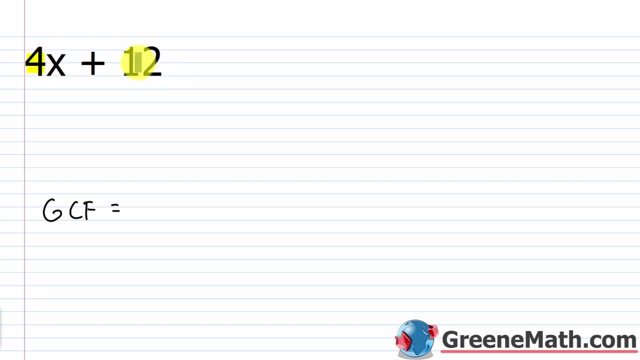 And this one's very easy, because I think about 4 and I think about 12.. I know that 12 is divisible by 4.. 12 divided by 4 is 3.. So the greatest common factor here would just be 4, right 4 divided by. 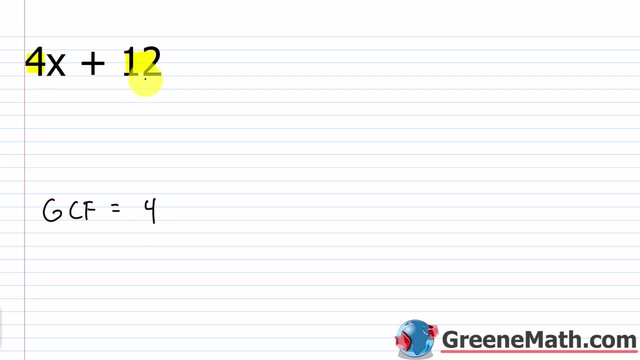 4 is 1.. 12 divided by 4 is 3.. And again, if you needed to see that you could break that down the long way, You could go. okay, well, 4 is 2 times 2.. And 12 is what It's 4 times 2.. So I'm going to. 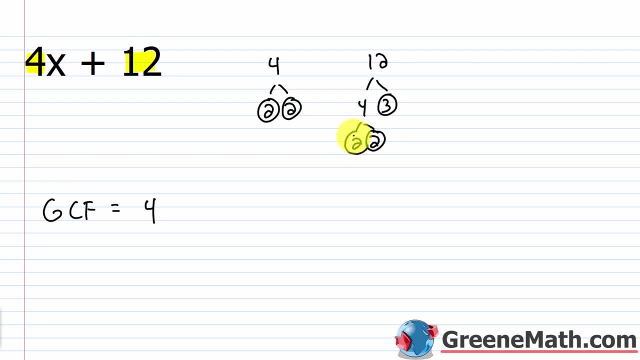 go 4 times 3.. 4 is 2 times 2.. So really I have 2 factors of 2 here and 2 factors of 2 here. So each one here is going to be divisible by 4.. So the greatest common factor is going to be a 4. All. 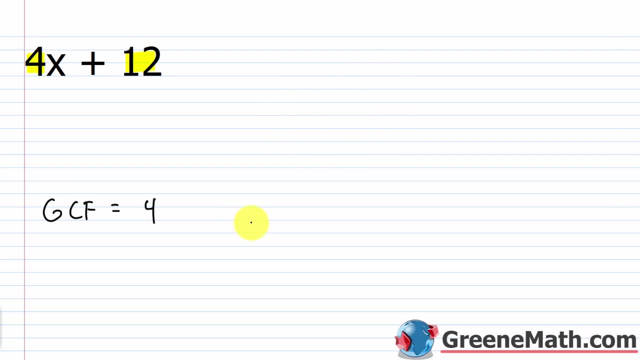 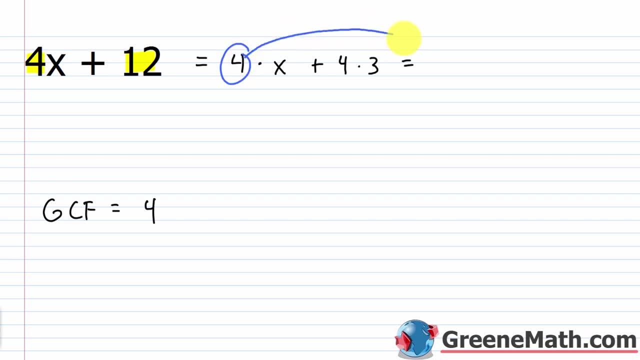 this would be equal to just pull the 4 out, place it outside of a set of parentheses And in the parentheses would have what's left. Here would just be an x Plus, here would just be a 3.. The other way you could think about that. remember, multiplication and division are opposites, So I 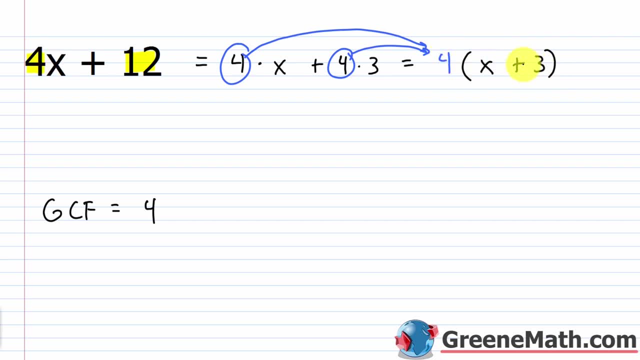 know, if I do 4 times x, I get 4x. I know if I do 4 times 3,, I get 12.. So I can reverse that and say here: well then, 4x divided by 4 would be what, That would be x. So that's going to go right there. 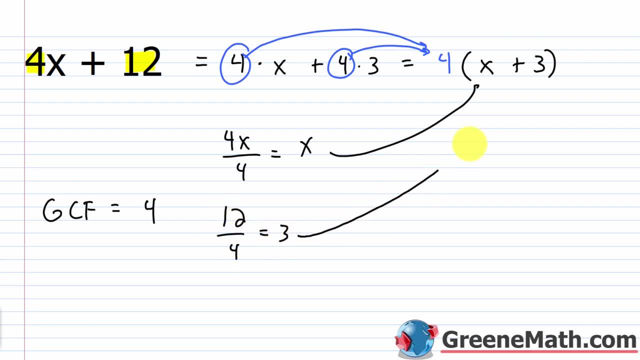 I could do 12 divided by 4, and that would give me 3.. So that's going to go right there, And I'm just thinking about multiplication and division as their opposite operations. So that's another way you can do that, And that's in fact what you're going to do when you do this mentally. 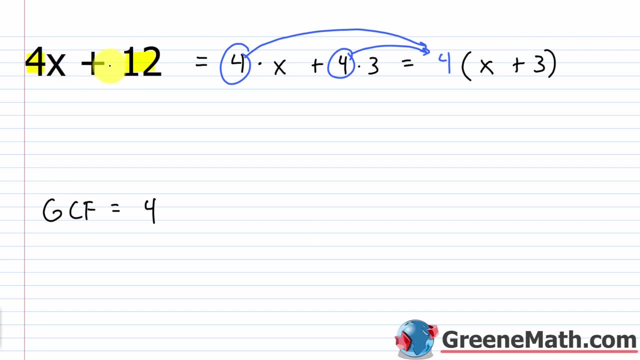 When I factor this now, I just look at it and I say, OK, well, I know that 12 is divisible by 4.. So 4 is the GCF First thing I come across. Then, after I put 4 outside of a set of parentheses, I would say: 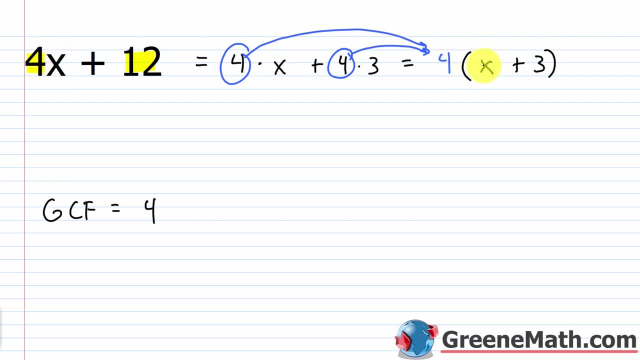 OK, well, 4x divided by 4 would be x. That's how I get my first term. Then I put my plus And next I say 12 divided by 4 would be 3.. That's how I get my second term there. All right, let's take 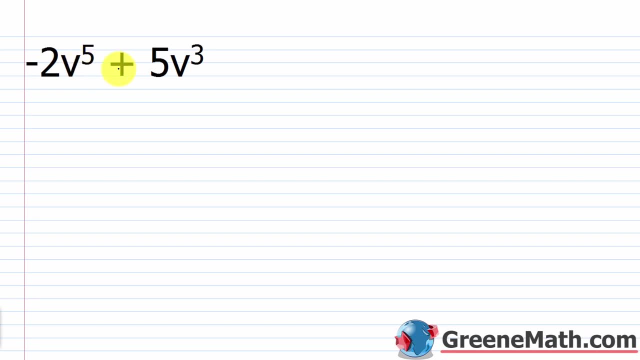 a look at another one. So I have negative 2v to the fifth power plus 5v cubed. So if I think about negative 2, it's just negative 1 times 2.. 2 is a prime number. 5 is a prime number. There's nothing common there number-wise. So in my GCF I'm not going to have a. 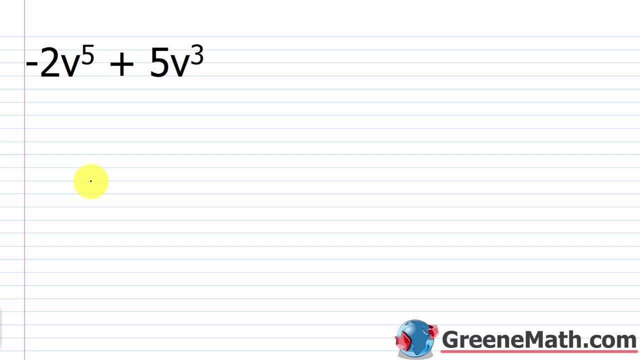 number involved other than I could use 1. And we'll talk about this later. I could also use negative 1 if I wanted to. I'm allowed to factor that out, But for right now I'm not going to think about any numbers. I'm just going to look at the variable. I have v to the fifth power and 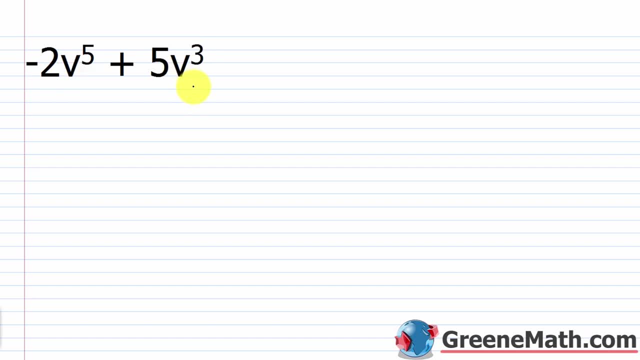 have v cubed, So everything has a v. The smallest exponent is a 3. So I know that's what I can factor out: a v cubed. So let's put equals. We'll put v cubed And then inside I'll have two spaces. here Again, I could. 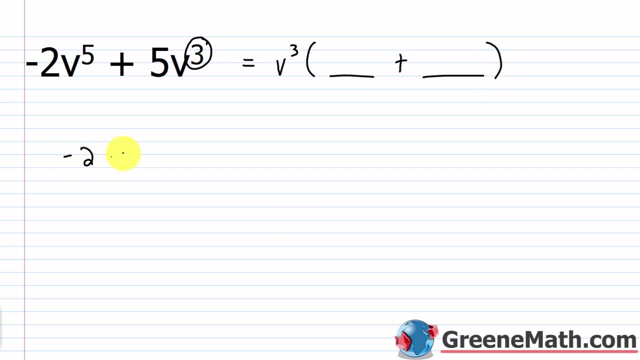 write this the long way and say I have negative 2 times v cubed, times v squared, plus 5 times v cubed. I could circle v cubed- Okay. a lot of students like to do this And say okay if I. 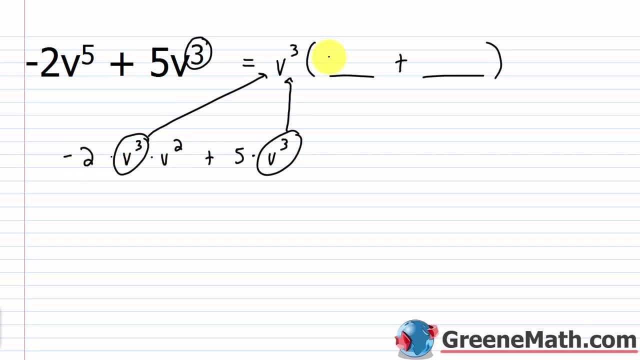 pulled that out, what's left? Well, here it's just negative 2 times v squared plus here it would be 5.. Okay, you can do it that way. Now another way. you can do this again, if I don't. 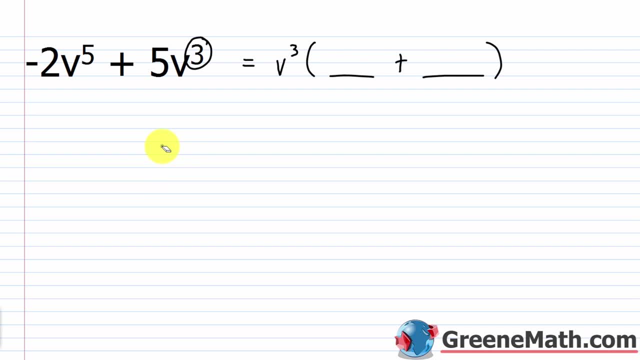 know what this is. let me just erase this. I can just use division. Okay, I could say: well, if I have negative 2v to the fifth power divided by v, cubed, what's that going to give me? It's going to. 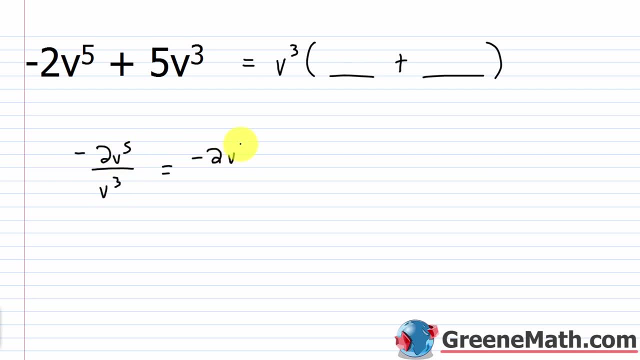 give me negative 2v to the fifth power of v cubed is v squared. That's what goes here: negative 2v squared. And I would do the same thing with this term. I would say: 5v cubed divided by v cubed is equal to what? Well, again, I have 5v cubed over. v cubed is 1.. So I'd get a 5.. 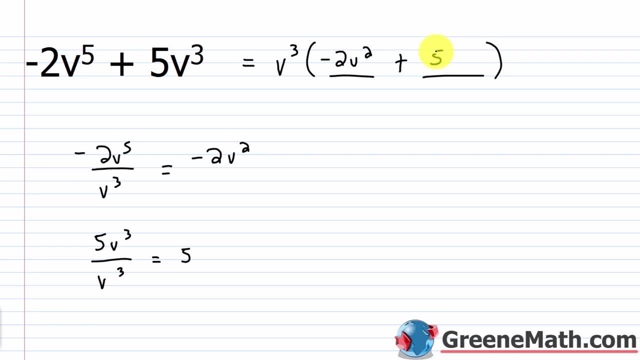 So you could use division, or you can kind of separate things with multiplication, where it's obvious what's going to be placed in here for these terms. Whatever is more comfortable for you. I can tell you that you're probably, as you get higher in math, going to use division, Okay. 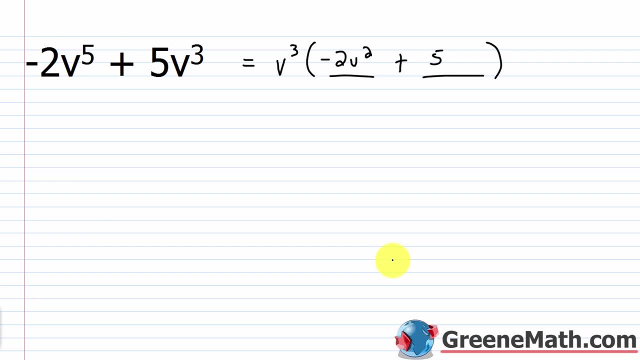 it's just easier to do that, It's more efficient And in most cases you're going to use division in your head. We know. if we wanted to check this, we could use our distributive property. v cubed times negative 2v squared would give me back to negative 2v, to the fifth power. 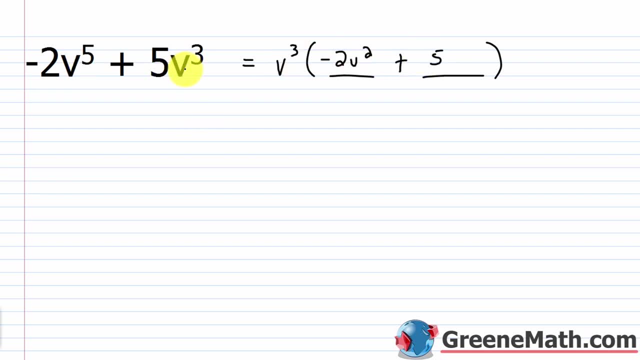 Then plus v cubed times 5 would be 5v cubed. So good to go there. All right, let's take a look at the next example. So suppose we have negative 8x cubed plus 12x. So we think about the numbers. 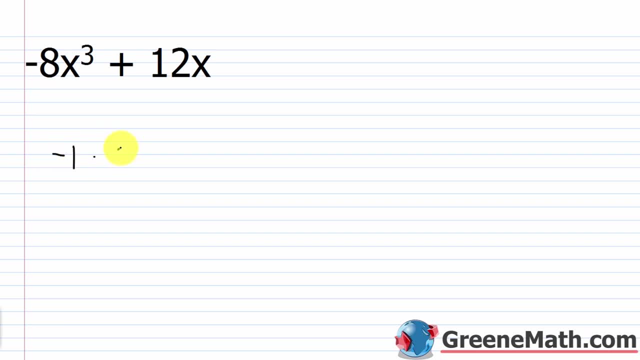 here I have negative 8, which I'm going to write as negative 1 times 8.. 8 is what I think about that, as Let's write negative 1 times 2 times 2 times 2.. We should know at this point that 8 is 2 cubed. 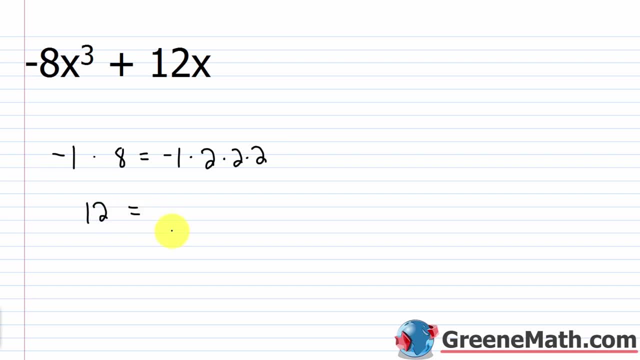 For 12, we have 1.. We have 4 times 3,, right, 4 times 3.. So 4 is 2 times 2, then times 3.. So kind of a quicker way to approach this would say: okay, well, I have negative 8 here, So just think about. 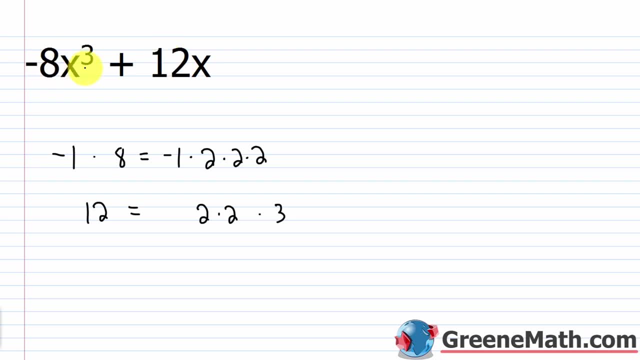 8 for a second, And then I have 12.. So both of those are even numbers And I would say: well, 12 breaks down into 4 times 3.. I know, 8 is not divisible by 3, but it is divisible by 4.. And so 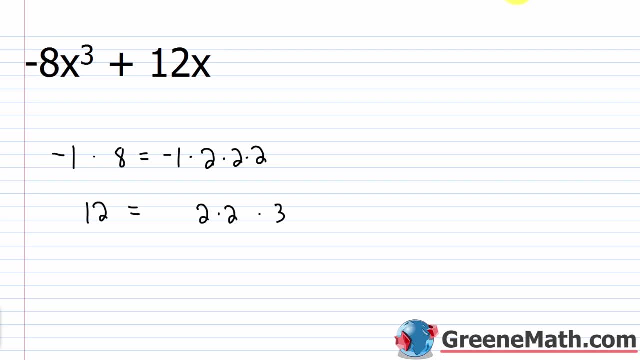 right away. I figured out that 4 is my GCF. But if you have to do this the long way for a little while, that's fine. You see that you have two factors of 2 there. two factors of 2 there, That's. 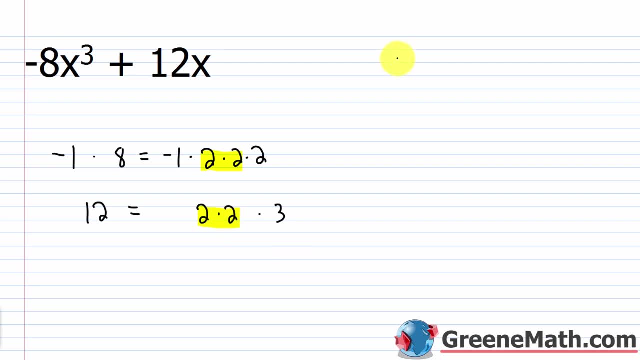 what's common, And 2 times 2 is 4.. So my GCF: here the number part, is a 4.. All right, for the variable part. we have an x cubed and an x to the first power. Again, it's common to everything. We go with the. 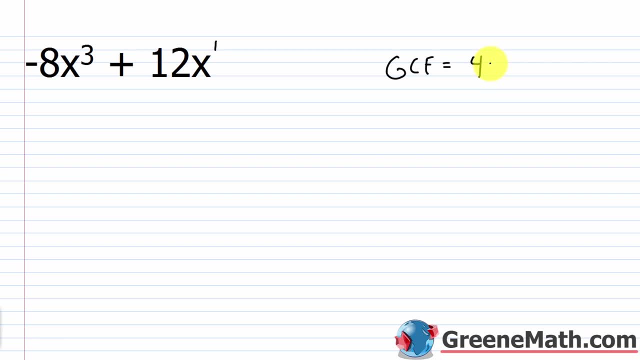 smallest exponent, which is 1.. So this is 4 and then x. All right, so if we want to pull this out, we would say this is equal to- and let me kind of scooch this down- We'll put our 4x outside of a set of parentheses. 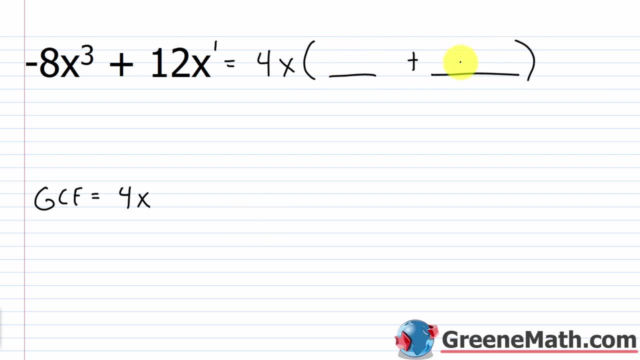 Put my two spaces in there. What goes here and here? Let's just use division. Okay, let's just use division. So if I had negative 8x cubed divided by 4x, negative 8x cubed divided by 4x, negative 8 divided by 4 is negative 2.. 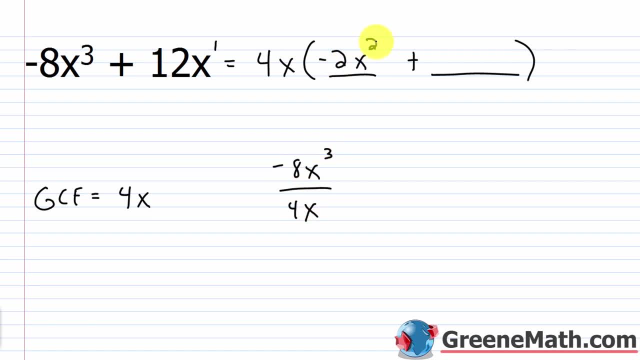 And then x cubed over x is x squared. Okay, And with that, next let's use 12x And let's divide that by 4x. We know that 12 over 4 is 3.. x over x is 1.. So this is a 3 here. 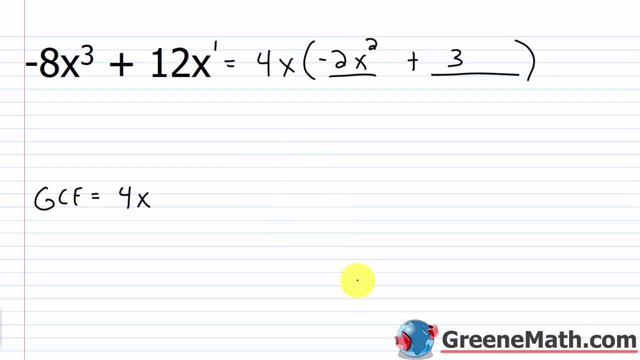 Okay, And again, if you use multiplication you'll get back to this: 4 times negative, 2 is negative, 8.. x times x squared is x cubed. Then plus, we have 4x times 3.. 4 times 3 is 12.. x comes along for the ride. You get 12x. 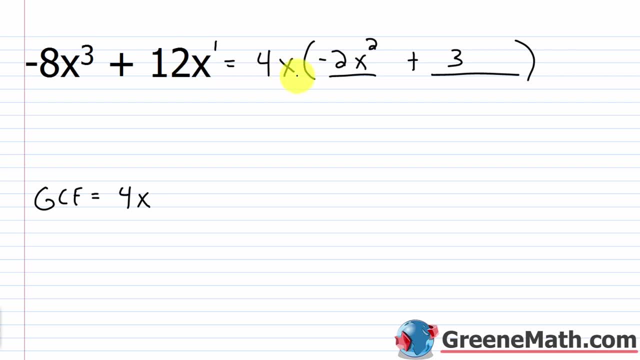 back. So our answer here is correct 4x times the quantity negative, 2x squared plus 3.. All right, let's take a look at another one. So we have 8x to the sixth power, plus 80x to the. 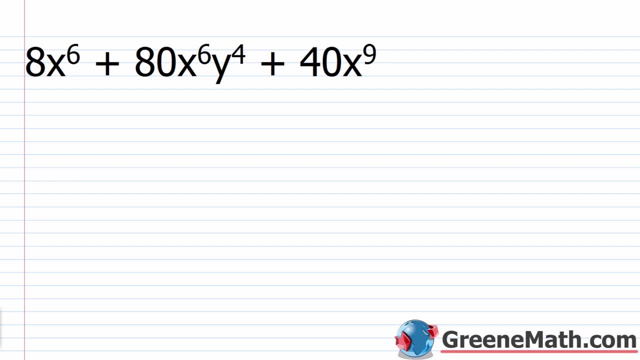 sixth power, y to the fourth power plus 40x to the ninth power. So I want you to kind of eyeball this And I want you to, without doing a prime factorization, pause the video and see if you can figure out what the GCF is. I think that you can do that, Okay. So I'm going to assume that. 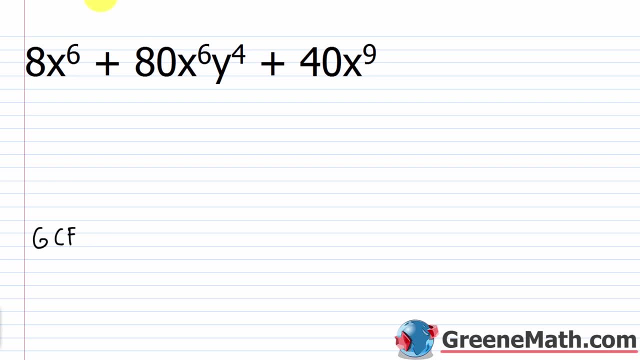 you tried that And really the method that I would use. I would see that I have an 8 here, an 80 here and a 40 here. Everything you should notice here is divisible by 8.. 8 divided by 8 is: 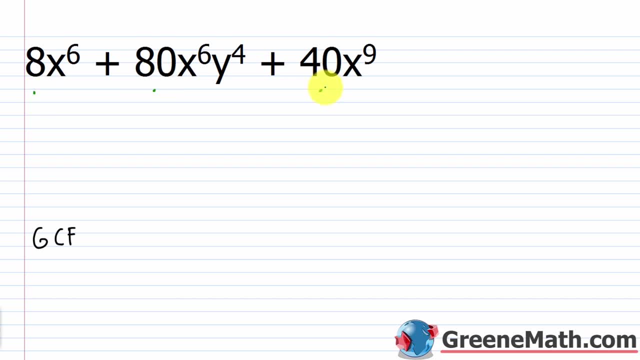 1.. 80 divided by 8 is 10.. 40 divided by 8 is 10.. 80 divided by 8 is 10.. 80 divided by 8 is 10.. 80 divided by 8 is 5.. So that tells me right away that the GCF, the number part, at least. 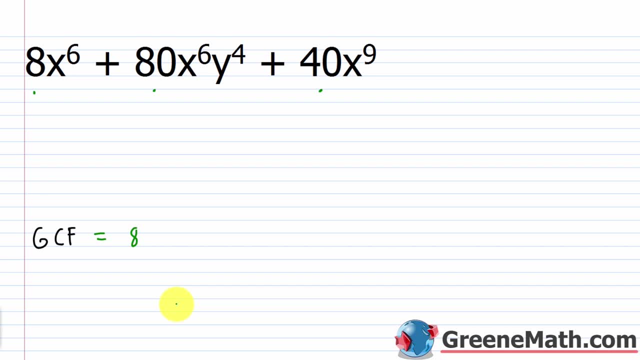 will be an 8.. Now for the variable part. I have an x, an x and an x. I have a y here, but I don't have a y anywhere else. So the GCF will only contain an x And then the smallest. 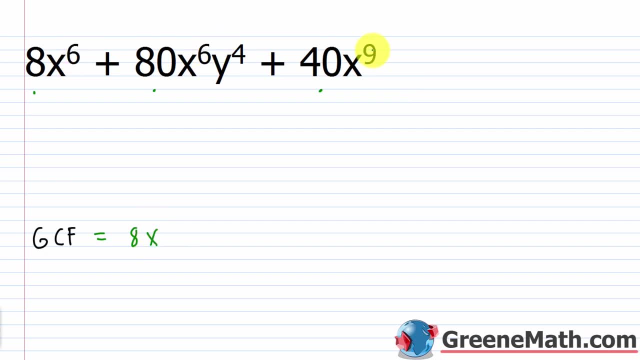 exponent is a 6, right, I have a 6 there, a 6 there and a 9.. So 8x to the sixth power is my GCF. So to factor this, let's put equals. Put 8x to the sixth power out in front And inside the parentheses. I'm going to have three spaces. 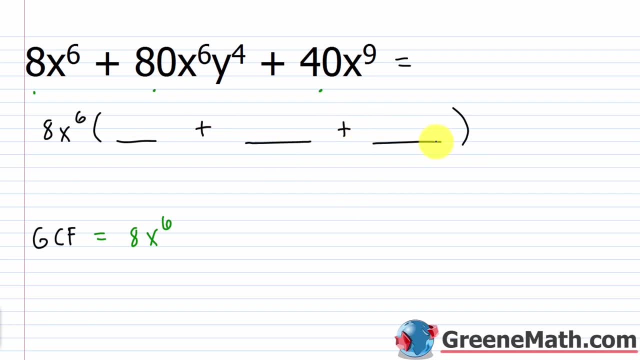 So what's going to go here, here and here? Well, all I'm going to do is I'm going to take that GCF and I'm going to use it as the divisor of each term here. So, in other words, I would start out with 8x to the sixth power and I would divide it by 8x to the sixth power. 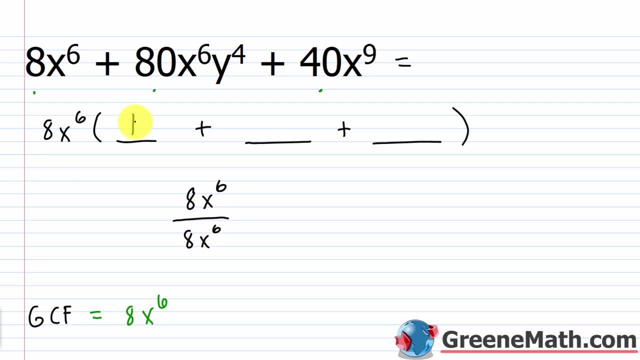 Of course 8x to the sixth power. over 8x to the sixth power is 1.. And next we'd have plus, minus. So I'd move to this next term. I'd have 80x to the sixth power, y to the fourth power. 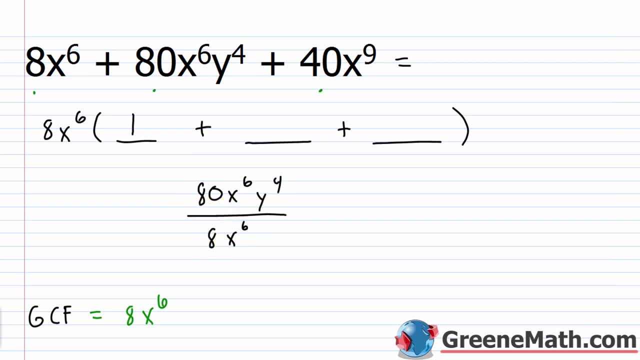 divided by 8x to the sixth power. So I know that 80 divided by 8 would be 10.. So a 10 would go there. x to the sixth power, or x to the sixth power is 1.. And then you'd have y to the fourth. 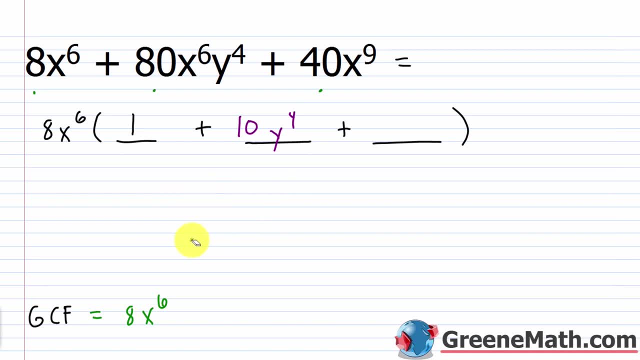 power. All right, let's do one more. here We have 40x to the ninth power, So 40x to the ninth power. We're going to divide that by again the GCF of 8x to the sixth power. We know that 40 divided by 8 is 5. x to the ninth power. 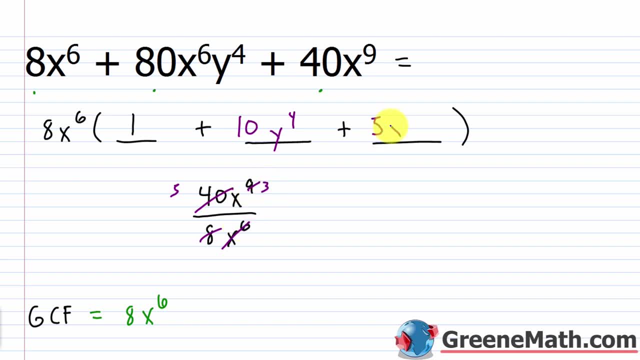 over x to the sixth power is x cubed. So this would be 5x cubed. Now you can check this if you want to. Again, you would use your distributive property and just kind of reverse this and you'll get back to this. All right, so our answer: here: we have 8x to the sixth power. 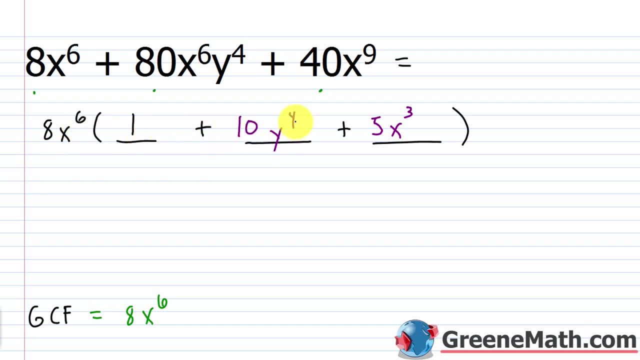 times the quantity We have: 1 plus 10y to the fourth power plus 5x cubed. All right, let's take a look at another one. Let's say you had negative 28x to the fourth power, y to the fourth power plus 24xy cubed plus 32xy squared. So again, if I think about the number, 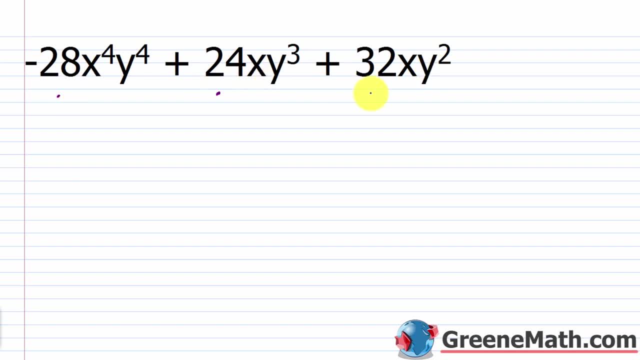 part here, without making a factor tree, without going through all that, just think about some things that we notice. The first thing I notice is that everything is an even number. So I know everything would be at least divisible by 2, okay. 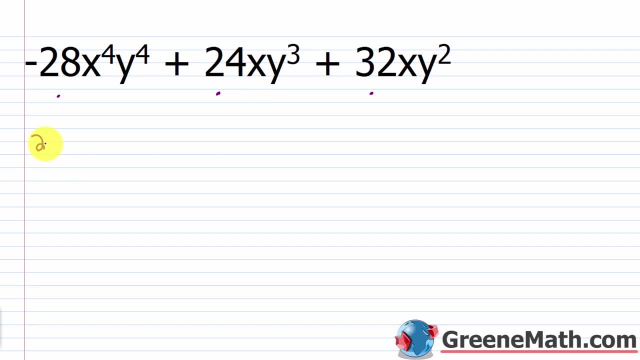 The next thing I would check and say: is everything divisible by 4?? Yeah, it is. Forget about this negative for a second Pretend, it doesn't exist. 28 divided by 4 is 7.. 24 divided by 4 is 6.. 32. 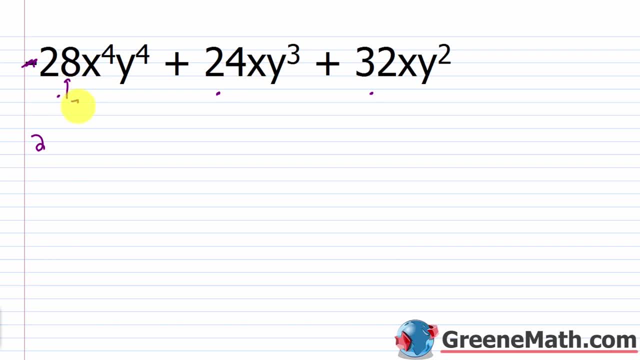 divided by 4, is 8.. The fact that this, divided by 4, is 7 is a big thing. 7 is a prime number, okay, So I know that I can't further break this down. It's just going to be 2 times 2 times 7,. 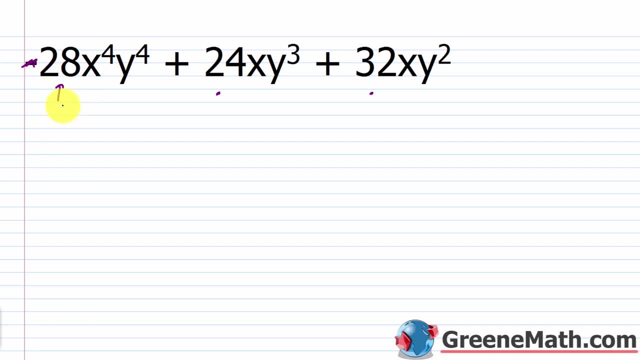 okay, So let me just write that right here real quick: This is 2 times 2 times 7.. And if I consider that negative, it's really negative: 1 times 2 times 2 times 7.. Now if this: 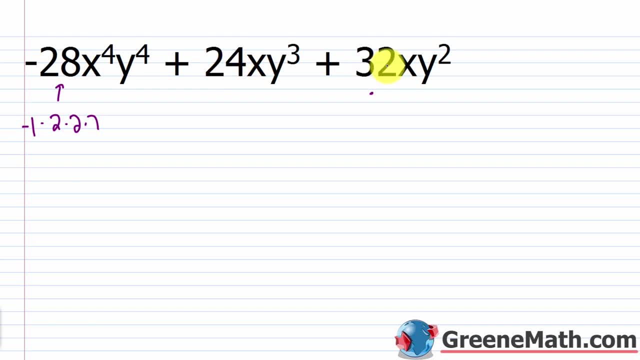 is not divisible by 7,, which it's not. and this is not divisible by 7,, which it's not. I'm done right. I know that everything will only have a 4 in common. okay, So I can stop and say my GCF. 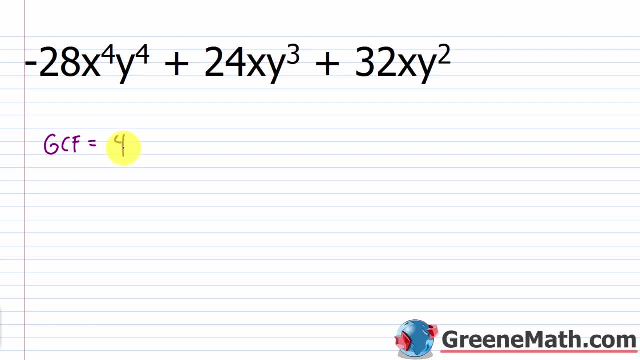 the number part at least, would be a 4.. And don't get me wrong: there's times where you get really big numbers and you have to make a factor tree. But if I consider that negative it's really You can't get around that. But in simple cases like this you should be able to eyeball these. 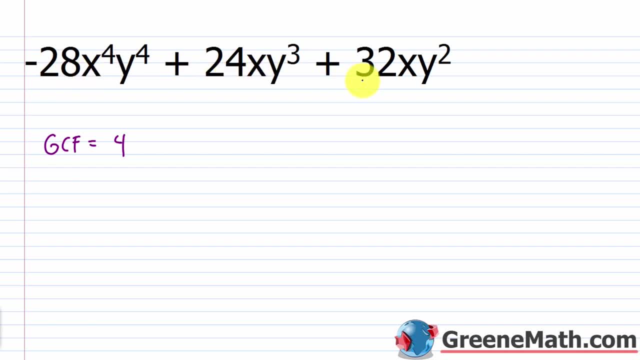 things and come up with your GCF, okay, And you're going to be expected to do that, especially as you move up and you start taking standardized tests. right, It's going to be built into the time limit, All right. So now I think about my variable part. I have an x everywhere and I have a y. 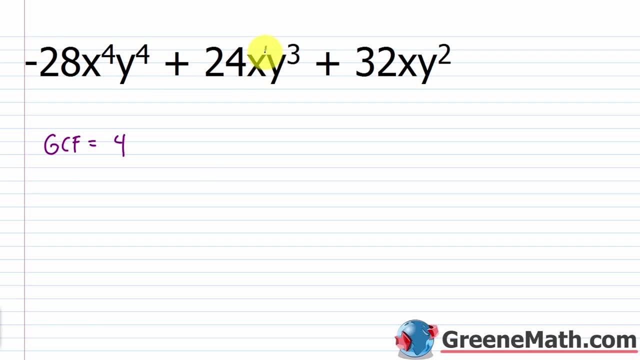 everywhere. So x, the smallest exponent would be a 1. So I'd put an x there And then for y, the smallest exponent would be a 3. So I'd put an x there And then for y, the smallest exponent. 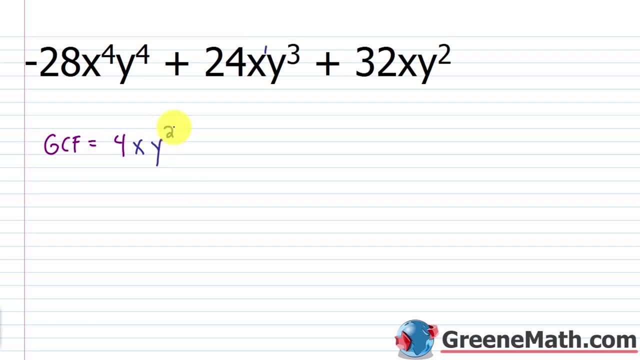 would be a 3.. So I'd put an x there. And then for y, the smallest exponent would be a 3.. So I'd put an 2.. So I'd put y squared. So my GCF is 4xy squared. All right, So if I want to pull that out, 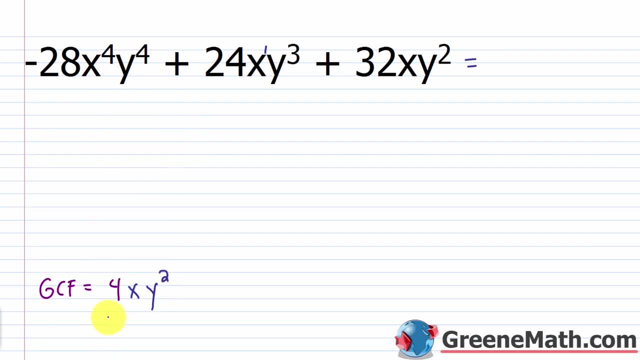 let's kind of scroll this down. Let's put equals, which we already did, And then 4xy, squared outside of a set of parentheses, And we'll have three terms in here. And again, to get the terms, I just take each term and I divide it by the GCF and I get the term right, Because, again, 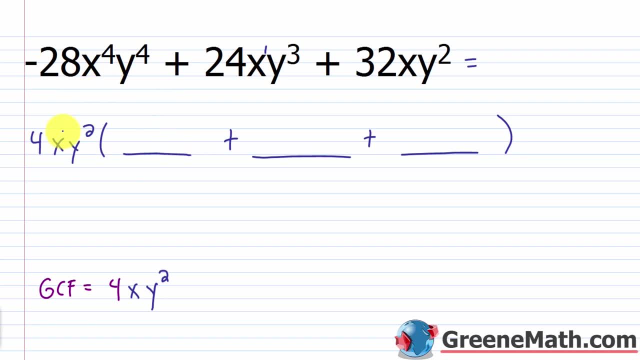 division is the opposite of multiplication. So if I multiplied I'd go back to what I had. So negative 28, x to the fourth power, y to the fourth power, divided by 4xy, squared, We think about negative. 28 divided by 4 is negative. 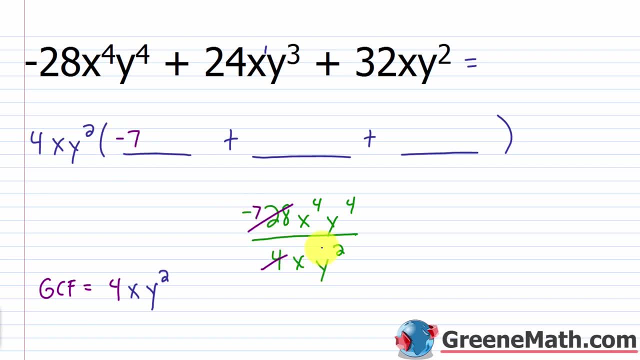 7. So this is negative. 7. We think about x to the fourth power over x. This is x cubed. We think about y to the fourth power over y squared: This is y squared. So this would be negative. 7, x cubed, y squared. All right, For the next one. 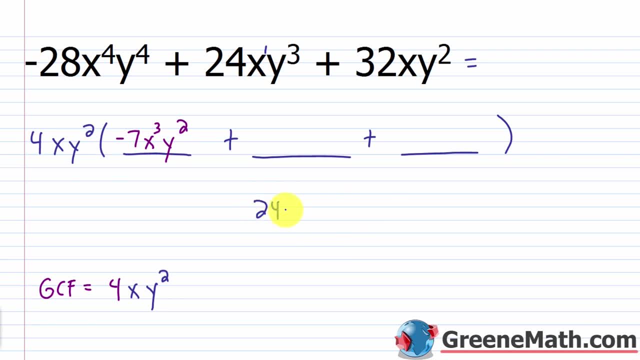 we have 24xy cubed over, we have 4xy squared. Okay, So let's look at this: 24 divided by 4 is 6.. x over x is 1.. y cubed over y squared is y to the first power. 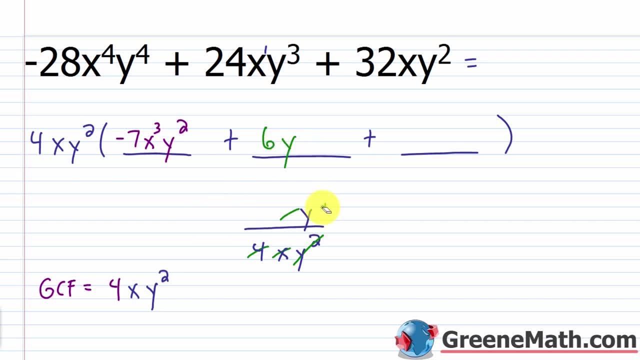 So this is 6y And let's erase this And we'll do our last one now. So we have 32xy squared over 4xy squared. So 32 divided by 4 is 8.. x over x is 1.. y squared over y squared is 1.. 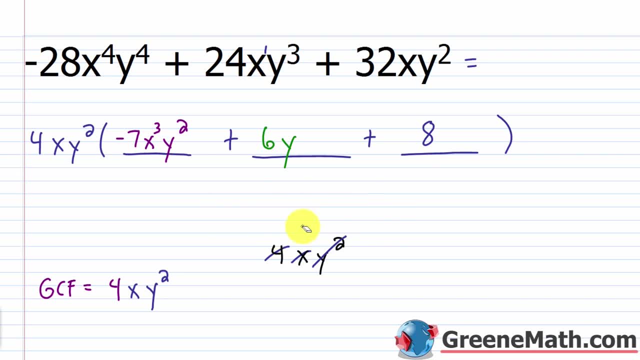 So I'm going to put an 8 there, All right? So let's erase this real quick. And we see our answer is 4xy squared And we're going to put an 8 there. So we're going to put an 8 there. So we're going to put an 8 there. 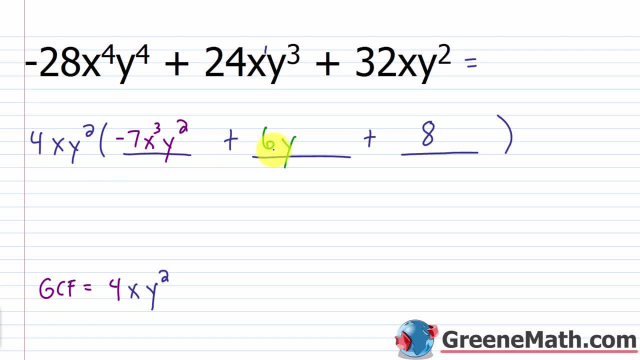 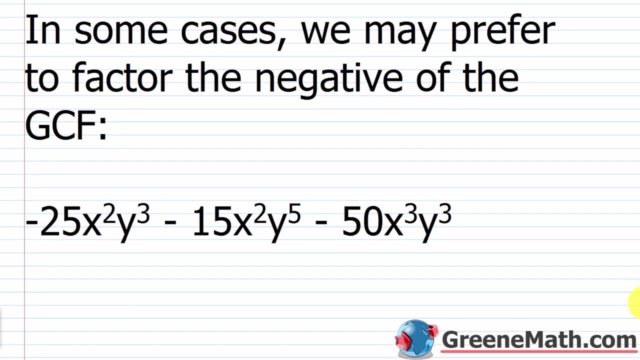 We have negative 7x cubed y squared plus 6y plus 8.. Now, if you wanted to check to make sure that you factored this correctly, you could use your distributive property and distribute this 4xy squared to each term And you could see that you get this polynomial up here back. All right, So. 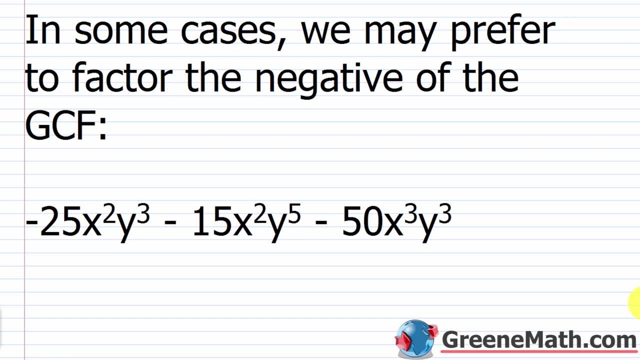 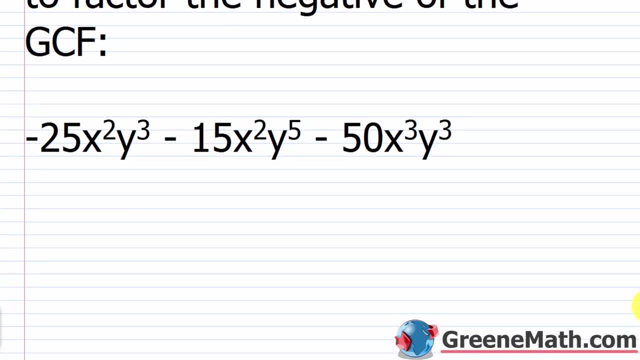 the next thing I want to talk about. we have here that in some cases, we may prefer to factor the negative of the GCF. So this is something that might be very useful for you, And if you want to use the factoring property, we are able to do so. In fact, in the next section when we start. 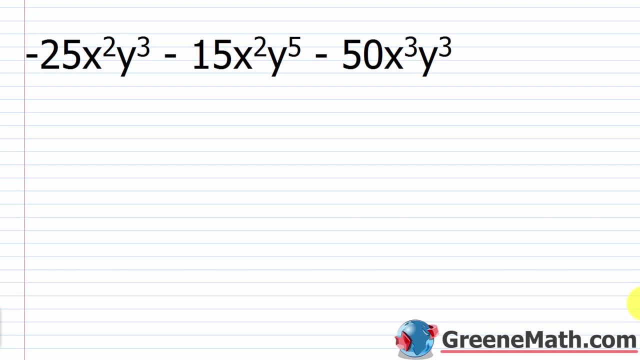 reviewing, factoring, by grouping, a lot of times we'll use the negative of the GCF to end up with a common binomial factor. So when we talk about pulling out the GCF, we could do the GCF or the negative GCF And it's still the same thing in terms of getting the correct answer. OK, so if I 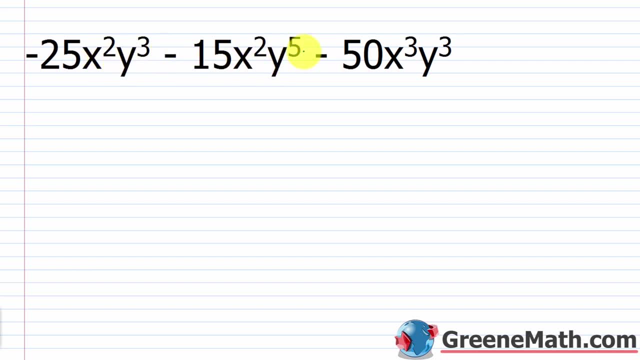 look at something like this: we have negative 25x squared over y cubed. negative 15x squared over y to the fifth and negative 50x cubed y cubed. I could pull that negative 15x squared over y to the. 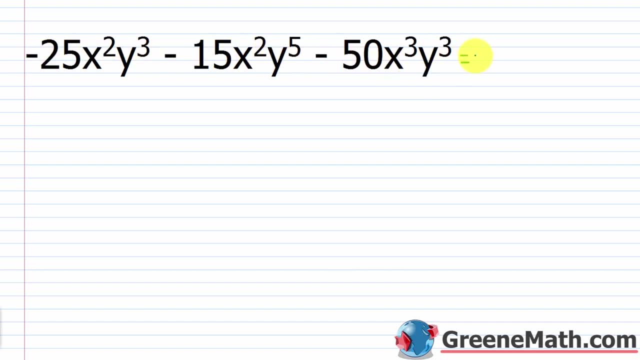 fifth And that's going to give me negative 15x squared over 1 to the fifth and negative 50x cubed y negative out to start. okay, if I want to. When I do that, I'm going to have the negative GCF. 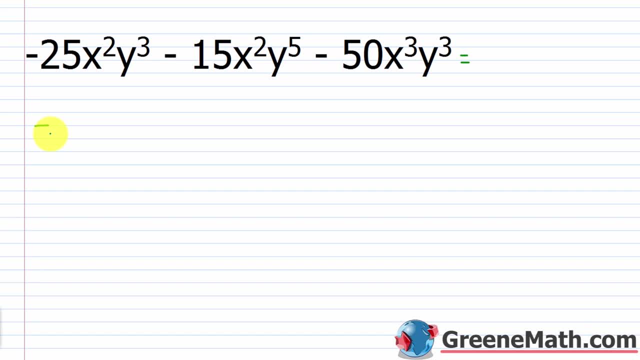 not the GCF itself, right? When we think about the greatest common factor, we know that the positive version is larger than the negative version, So that's why we say the negative of the GCF when we do something like this. Now, if I think about what the GCF is here, think about 25,. 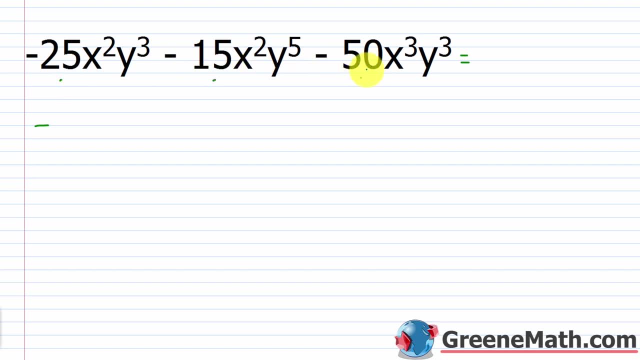 15, and 50. They're all divisible by five, right? 25 divided by five is five. 15 divided by five is three. So I can stop there. I don't even need to go there. I know that these two only share a common 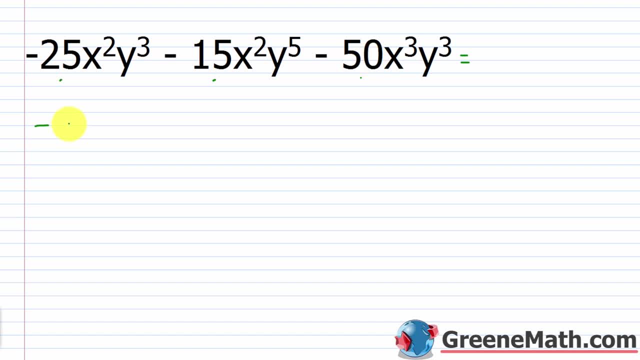 factor of five, And this one also has a factor of five, So I can just put five down. Again. if I'm doing the GCF, I want positive five, But because it's convenient, if I want to do the negative of it, I just do negative five. right, And both answers are acceptable. Now, when I think 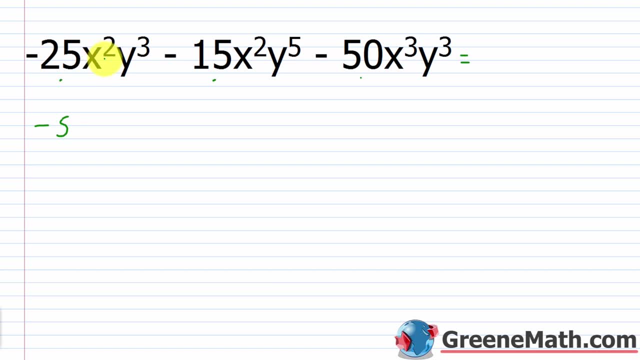 about the GCF. I'm going to have the negative of five. So I'm going to have the positive of five, The variable part. I've got x squared, x squared and x cubed, So the smallest exponent is a two. 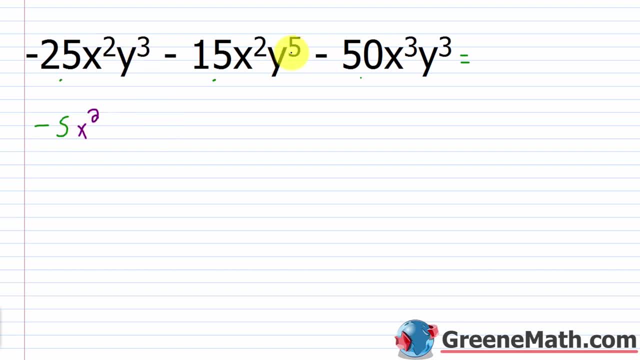 so I go with x squared. Then I've got y cubed. y to the fifth and y cubed. The smallest exponent is a three, so I go with y cubed. So inside the parentheses, now these won't be minuses anymore. 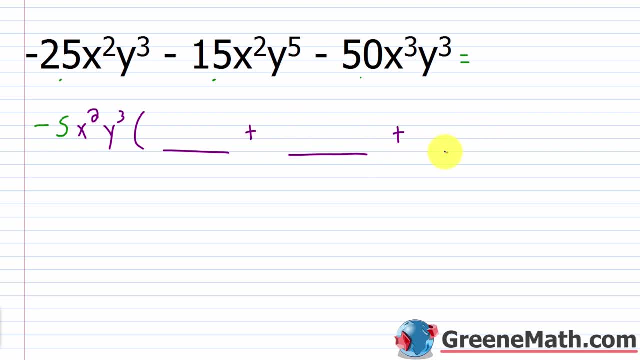 They'll be pluses. okay. And why is that the case? It's because I pulled the negative out right, So everything inside will now be positive, because negative times positive would bring me back to negative. Negative times positive bring me back to negative. Negative times positive. 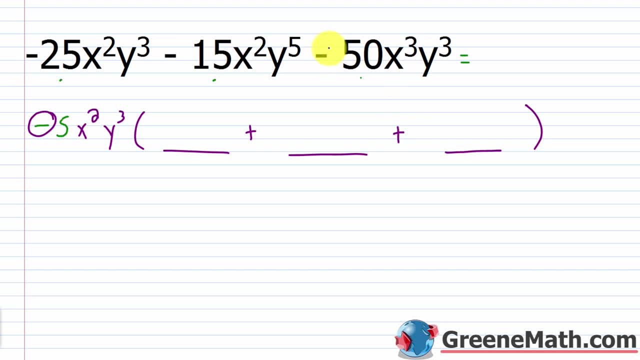 bring me back to negative. Very important: you understand how to deal with signs when you're factoring. okay, So I'm going to do some division: Negative: 25 x squared y cubed. divided by negative: five x squared y cubed, What do I get? Negative over negative again. 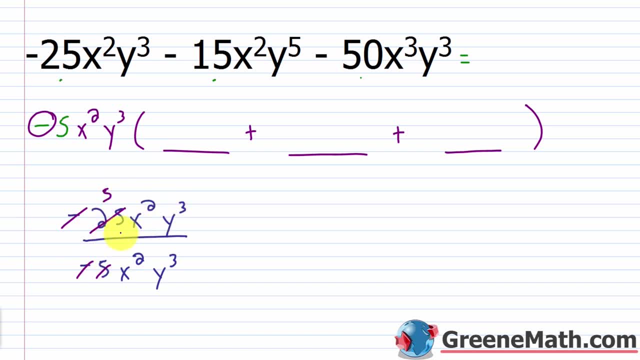 is positive, All right, 25 over five is five, and then these cancel themselves out. So this first position here is a five. For the second position, I would have negative 15 x squared y to the fifth, power over negative five x squared y, cubed. So negative 15 over negative five is going to give me positive. 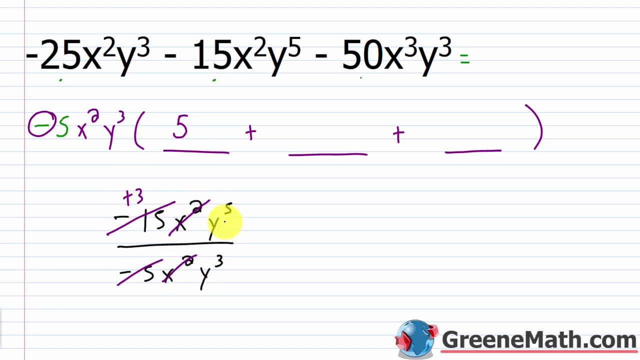 three: X squared over x squared is one y to the fifth, power over y cubed is y squared. So this would be a negative. So I'm going to do a zero and I'm going to do a mil, I'm going to do a five. 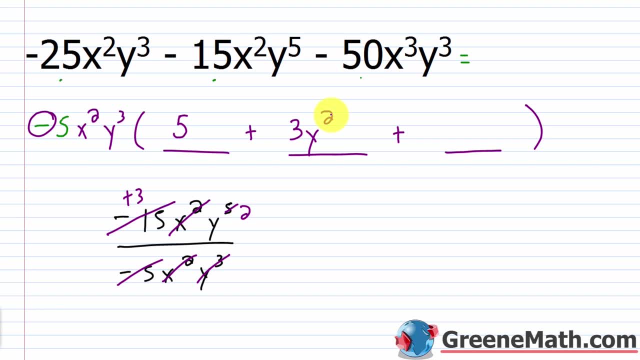 3y squared. And then, lastly, we would have negative 50x cubed, y cubed over negative 5x squared, y cubed, And so negative 50 over negative 5 is 10.. x cubed over x squared is x to the first. 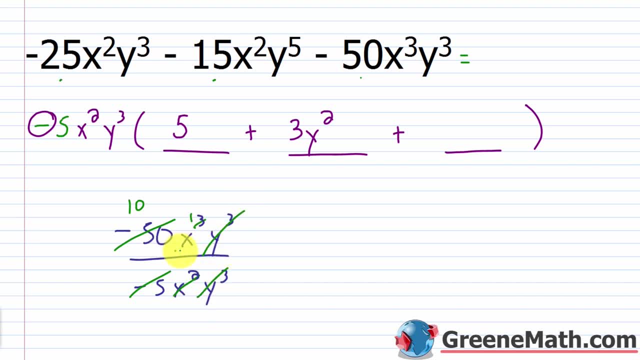 power: y cubed over y cubed is 1.. So this would be 10x, So 10x. Now, what you could have done again- this is what I'm trying to do here- is explain to you that I didn't have to factor out. 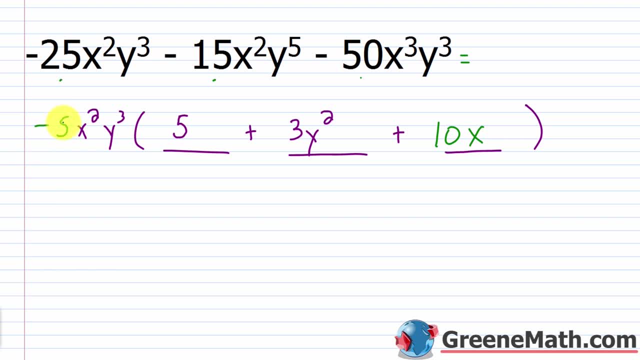 this negative. I could have said: the GCF is 5x squared, y cubed, So I could have just factored out a positive. The only difference is all the signs in here would change. This would be negative, this would be negative and this would be negative. So it's just a matter of preference. 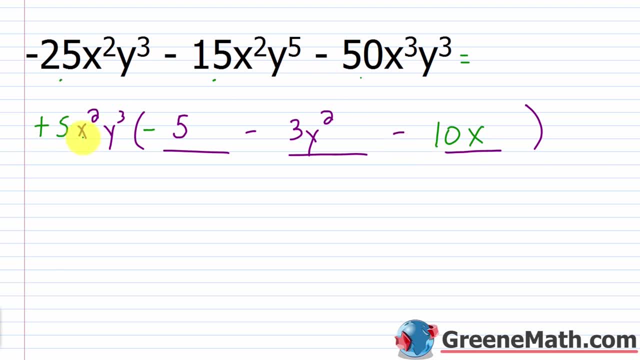 okay, What do you want it to be? If I wanted to pull the negative out, I'm allowed to do that. That's all I'm telling you. You could factor out the GCF or the negative of the GCF, and it's still going to be an acceptable answer either way. 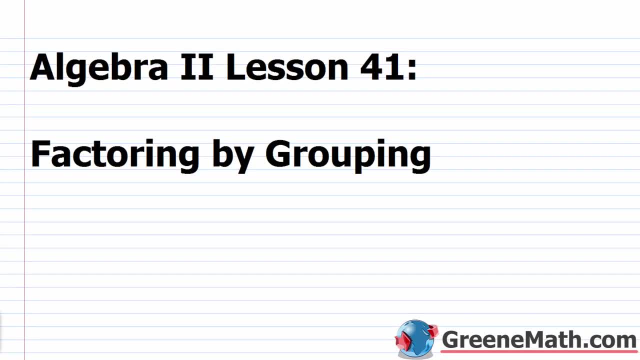 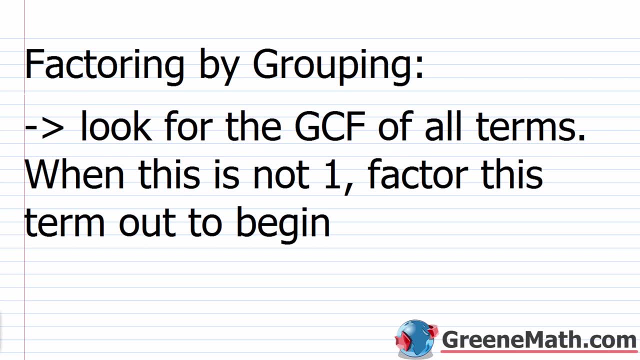 Hello and welcome to Algebra 2, Lesson 41. In this video we're going to learn about factoring by grouping. All right, so again, for most of you that took an Algebra 1 course, you've had experience with factoring by grouping. It's not a very difficult concept. 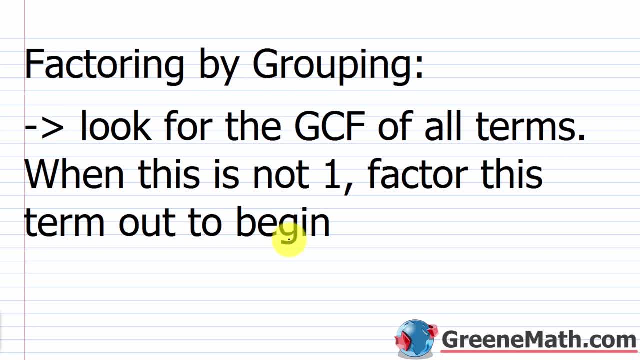 It's something you just have to do, enough practice with. So for factoring by grouping, the very first thing you want to do- you want to look for the GCF. Again, it's a common factor of all terms. Now, when this is not a 1, or we could also say when it's 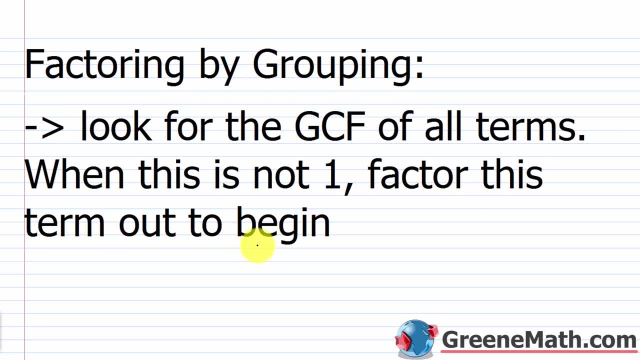 not a negative 1, you want to factor this term out to begin. So what are we saying here? Well, let's say, if we had a four-term polynomial and everything had an x as an example, Well, you'd want to pull that out before you even start doing anything, because that's common to 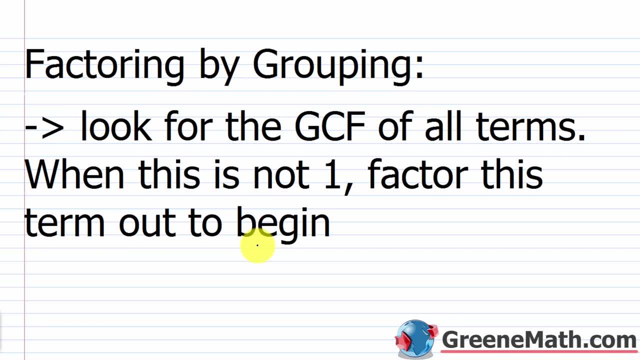 everything. When you don't do that, you're going to end up with additional factoring after you do the process and you might miss it. Okay, and that's going to give you only partial credit on your test, your homework. 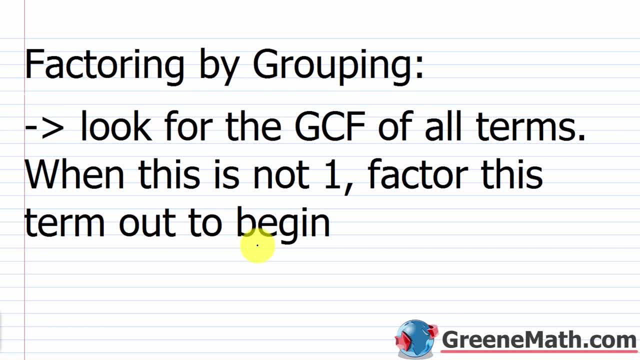 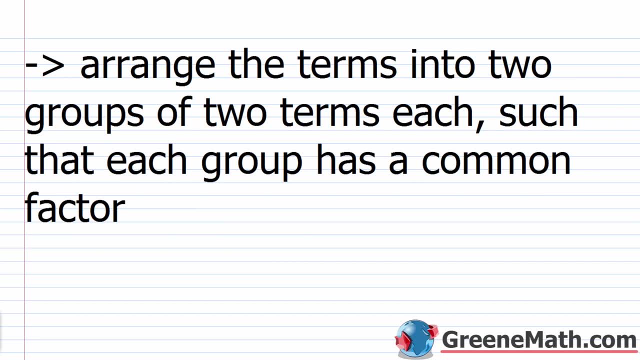 whatever you're working on, So you want to always make sure you pull things that are common out first before you go into the steps. All right, now here's the next part, and this is where it gets a little confusing. You want to arrange the terms into two groups of two terms each, So this: 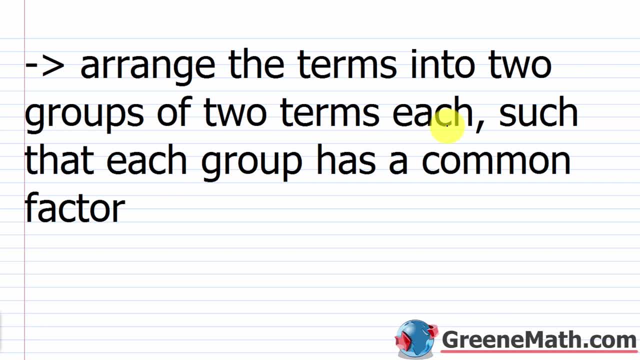 is for a four-term polynomial, So you'll have group 1 and group 2.. Now I have such that each group has a common factor. Now, in some cases, that common factor might be one or negative one. The whole goal is to end up. 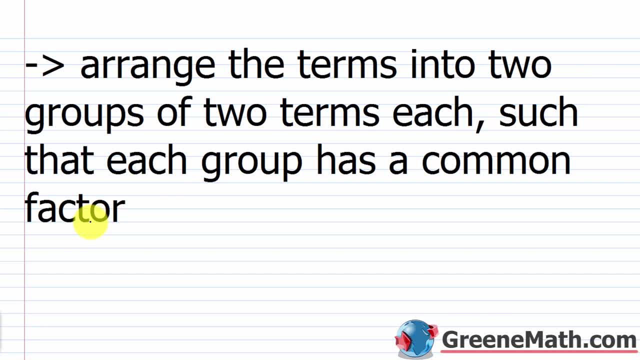 with a common binomial factor. Okay, so you're going to have to play around with this a little bit. This isn't something where you can just kind of read a procedure and it's always going to be the same. So I have here that you'd factor the GCF out of each group. Again, that might be. 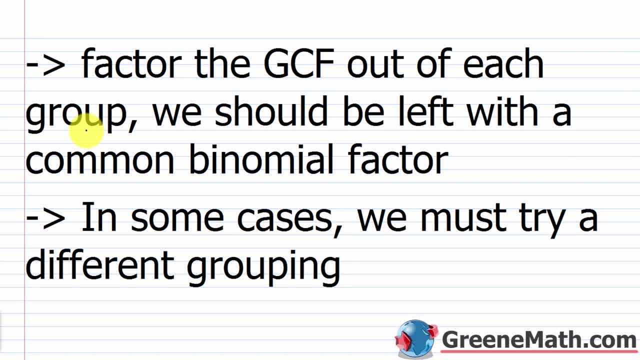 factoring out something that's not one from one group. It could be factoring out one from another group, And I have here. we should be left with a common binomial factor. Now, if you try a certain configuration and it doesn't work- I have here: in some cases we must try a different grouping. 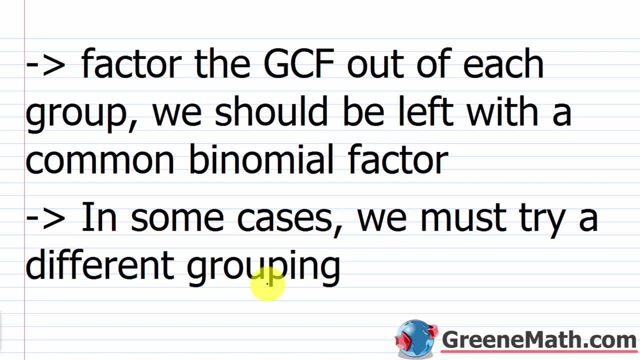 So don't get discouraged right away or don't say, oh, this isn't factorable right away. A lot of the problems you're going to see, especially if you're in a section of factoring by grouping, are going to be factorable. You just have to change around the terms. 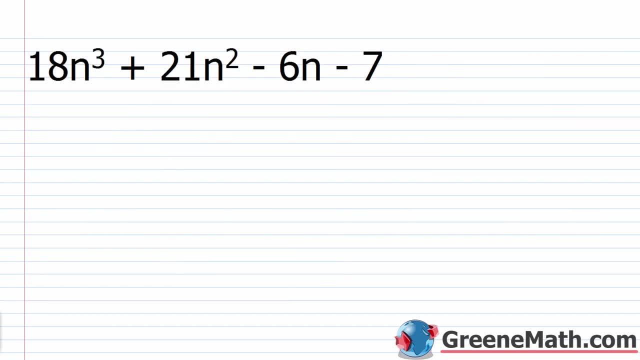 Let's look at the first example, and this one's pretty easy. I'm going to start out by just going with the way things are presented and I'm going to show you that you can do this multiple ways. So we have 18n cubed plus 21n squared, minus 6n minus 7.. So again, the first thing I want to. 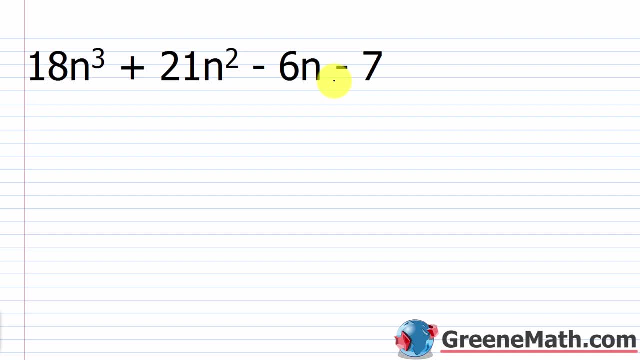 think about is: is there something other than 1 or negative 1 that I could pull out from every term here? set it outside of some parentheses. The answer to that is no, And what I look for right away I see this 7 here. The 7's a prime number, so I know that it's only divisible by itself. 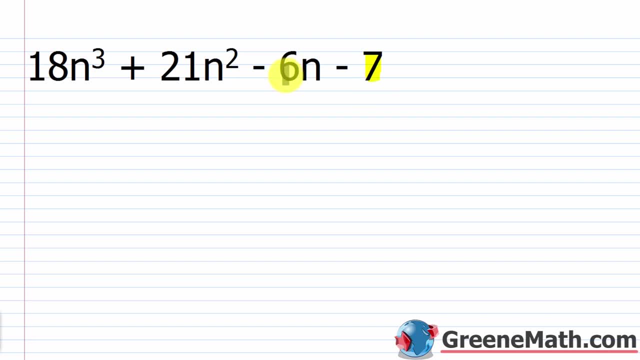 or 1.. Could I pull a 7 out from this 6?? No, 6 is 2 times 3.. So I can just stop there. I know I'm not going to be able to pull a number again other than 1 or negative 1 out from every single. 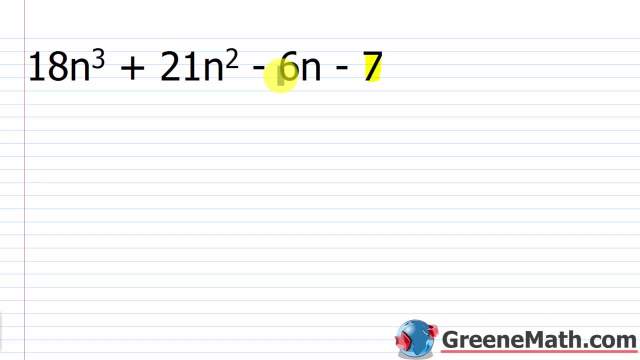 term of this polynomial Now, variable-wise, you see that you have an n, an n and an n, but I don't have an n here, so that's not going to work either. So we're not going to be able. 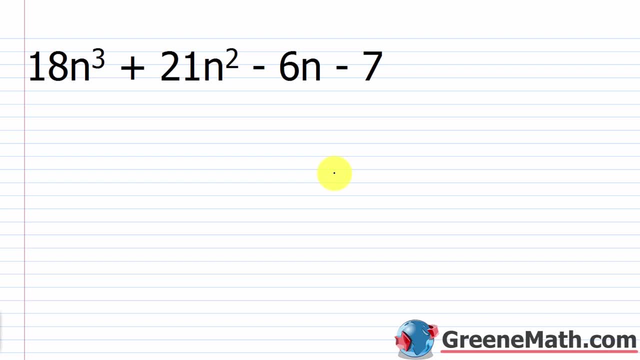 to pull anything common out to start, All right. so then we kind of go into our grouping. So I think about the first two terms as a group, So we could say this is, you know, group 1.. And then I think about 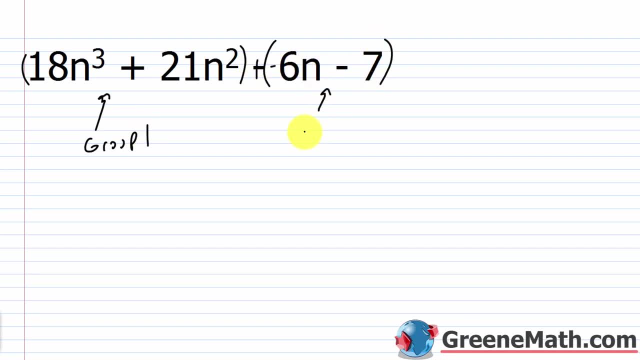 the next two terms as a group. So let's say this is group 2.. So in the first group or group 1, what could we pull out? Let's just say this is a separate problem and we go back to what we were. 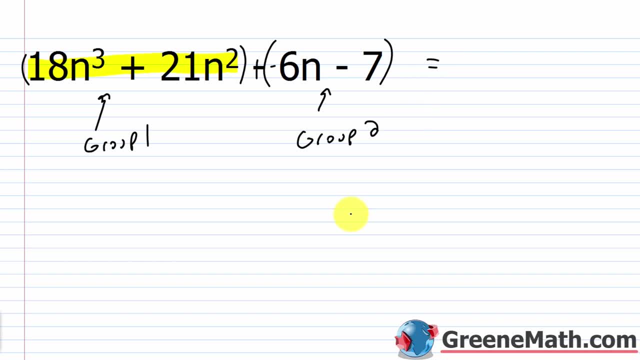 learning in the last video where we factored out the GCF. Well, if I think about 18 and 21,. they have a common factor of 3, right, 21 divided by 3 is 7.. 18 divided by 3 is 6.. And 6 is 2 times 3,. 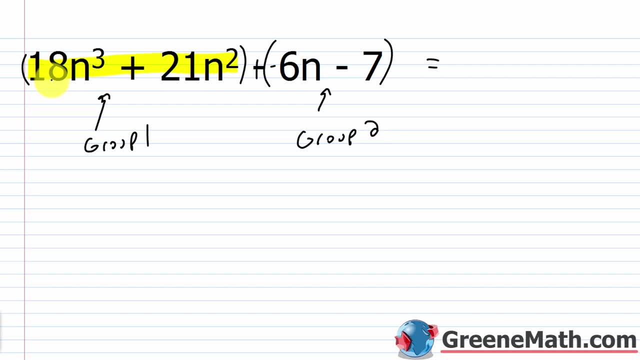 so I can't go any further. So if I pulled out a 3 and put that out in front and then variable-wise I have n cubed and n squared, The variable is the same. so I know I'm going to have an n. 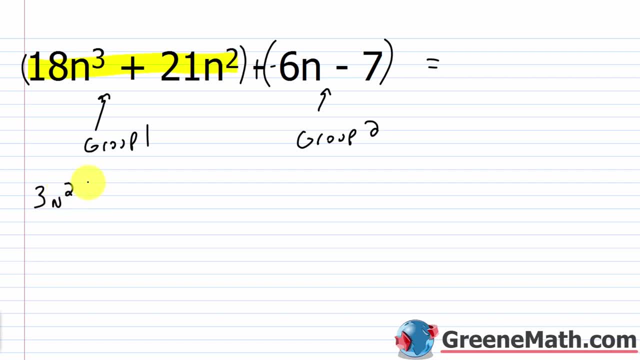 And the smallest exponent is a 2, so it would be squared. So let's say I pulled that out from that first group. What's left? The 2 terms inside? now, Remember we can use division: 18 divided by 3 would be 6.. n cubed. 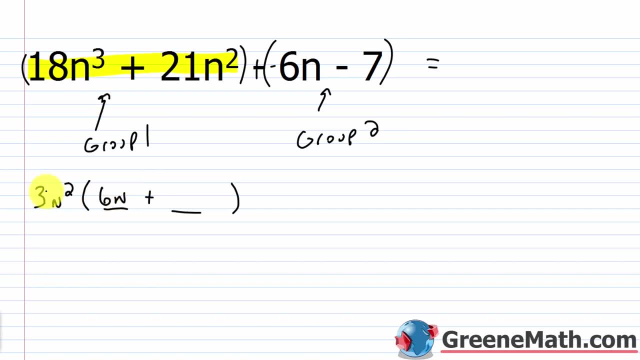 divided by n, squared would be n. Then 21 divided by 3 would be 7.. n squared over n squared is 1.. So I factored the GCF out from group 1.. I've written it like this. Now I'm going to put plus. 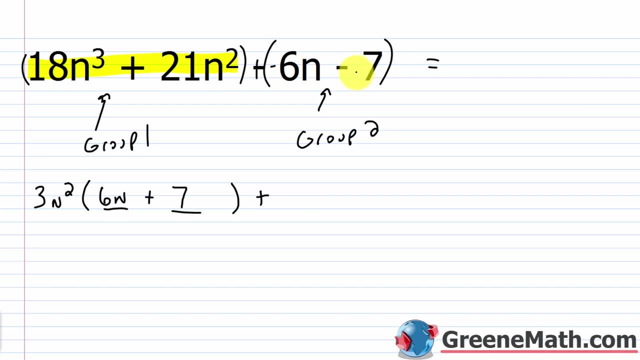 From group 2, negative 6n minus 7,. what could I factor out? What's the GCF there? Well, 6 and 7, you're not going to get anything. You're going to get nothing out of there other than 1, or you could do negative 1.. You can't do. 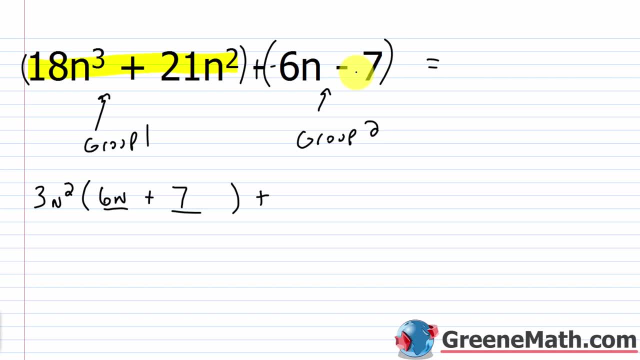 anything. 7 is prime, 6 is 2 times 3.. The n is only part of this. negative 6n. There's no n over here, So in this particular case I'm going to try 1, and then I'm going to try negative 1 to. 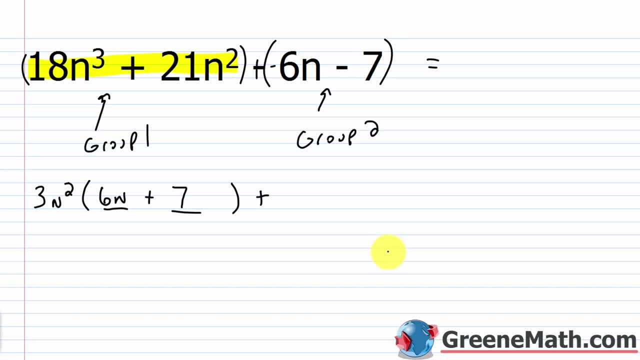 see if I end up with a common binomial factor. It's obvious, because the signs here are positive and positive, that I need to pull out a negative 1, because this is a negative and this is a negative. So if I pull out a negative 1, I'm going to get a negative 1.. So if I pull out a negative 1,, 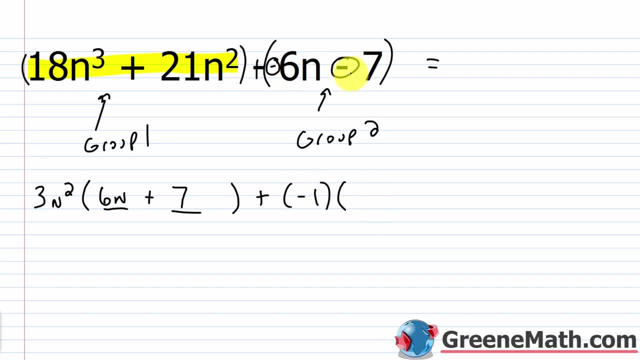 what's going to happen is the sign of each term in here is going to change. Negative 6n divided by negative 1 is 6n. Negative. 7 divided by negative 1 is positive 7.. So now, if you look, we have the. 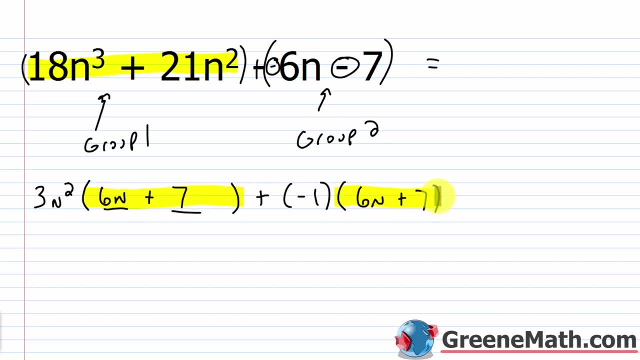 quantity 6n plus 7 and the quantity 6n plus 7.. So we have a common binomial factor And, just like when we factor anything else out, we can just pull it out. So we'd have 6n plus 7.. And if I've pulled that out, well then this is left here. So I'm going to start. 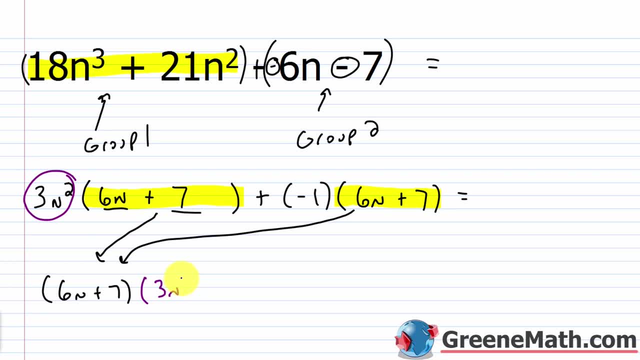 another set of parentheses and say: this is left. So 3n squared is left. Then I have my plus And I'm left with. if this is gone, I just have the negative 1.. So I can put plus negative 1, or most. 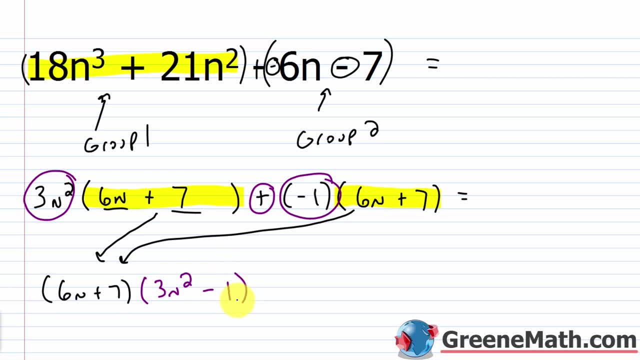 of you would just rather write minus 1.. It doesn't really matter. And I'm left with the quantity 6n plus 7 times the quantity 3n squared minus 1.. Okay, Very, very easy. Now I want to show you a different grouping and show you that there's 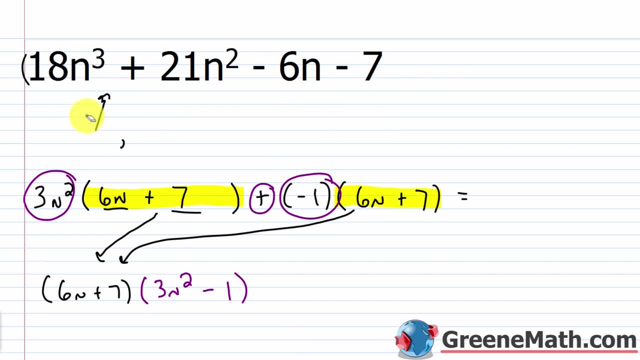 alternative ways to kind of get the same answer, And another thing you might want to do: you might want to pause the video and you might want to foil this and prove to yourself that it goes back to this. A lot of students have trouble believing that, So let me erase this as well, for right now. 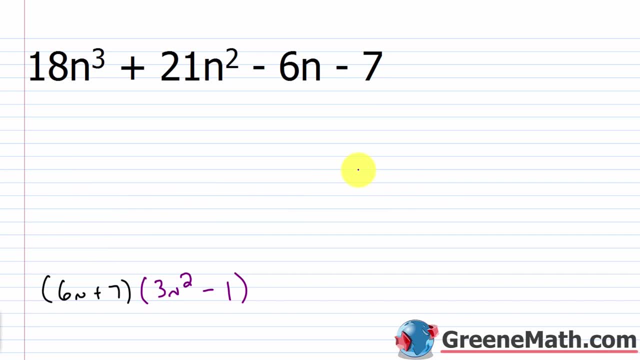 We don't need that anymore. And let's say, you started this problem out by saying: okay, well, I have an 18 here and I have a negative 6 here. Well, each of those would be divisible by 6. So those should be in a group together. Okay, Those? 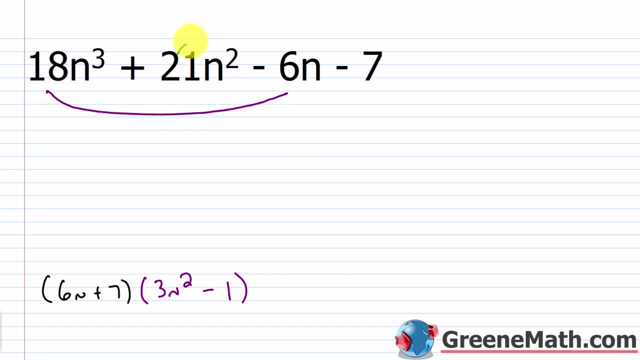 could be group 1,, for example, And then you might say: okay, well, this has 21 and this has a negative 7. Those could be a group, because each is divisible by 7.. Okay, So let's try it that way. 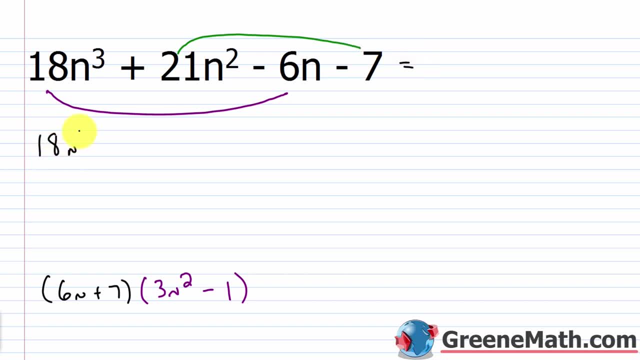 Let's make group 1: 18n cubed, Then you'd have minus 6n. Let's make group 2. We'll have plus 21n squared, minus 7.. So this would be your group 1. And now this would be your group 2.. So from group 1, now I can pull. 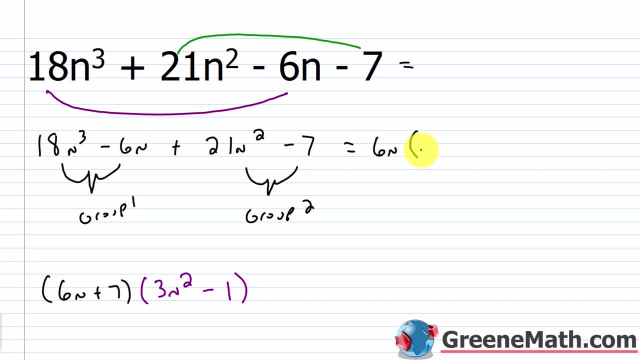 out a 6n. So if I pulled out a 6n, what would I have? Again, 18n cubed divided by 6n would be what That would be 3n squared, And then negative 6n divided by 6n would be negative 1. Then we'd have plus From group 2, I can pull. 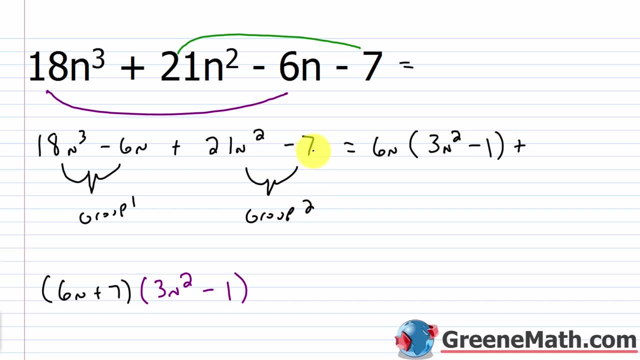 out a negative 7, or I can pull out just a 7.. And it's just a matter of the signs. Now, if you look at group 1 and what we pulled out, the binomial inside the parentheses is positive, then negative. 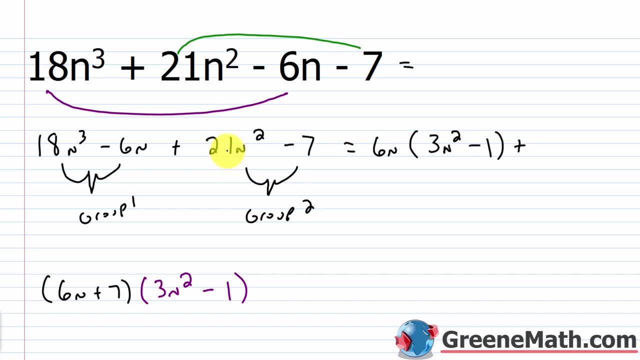 If I pull something out here, I'm going to want that same configuration. I want positive, then negative. So, seeing that I know I want to just pull out a positive 7.. So pull out a 7.. And what would happen? 21n squared divided by 7 is 3n squared Negative 7 divided by 7,. 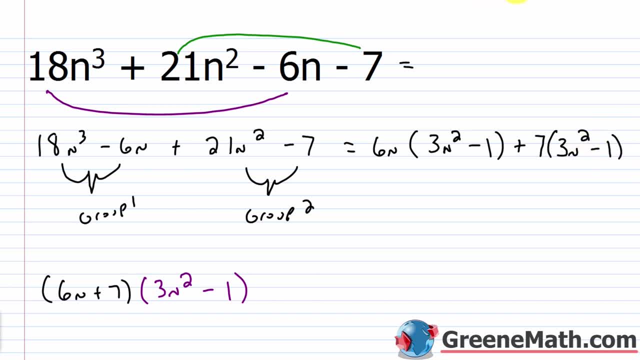 is negative 1.. So minus 1.. And again you get your common binomial factor of 3n squared minus 1.. Again, that's what you have right here. If I factored it out, I would get the same thing as I got here, right. 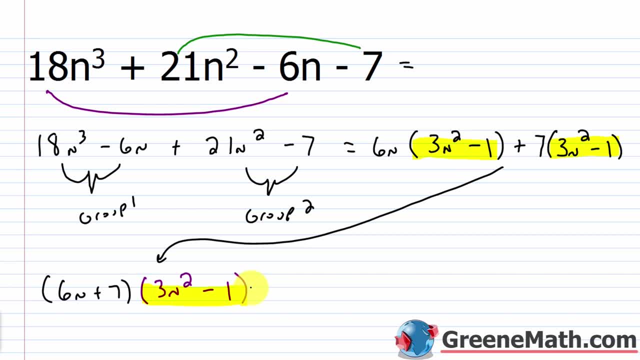 I'd pull out the 3n squared minus 1.. It would be there. It'd be in a different position. It'd be in the first position here, But that doesn't matter. The order of multiplication is irrelevant. Then I would have the quantity 6n plus 7 as my other. 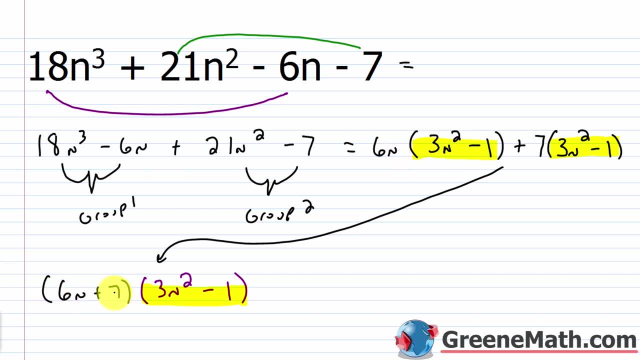 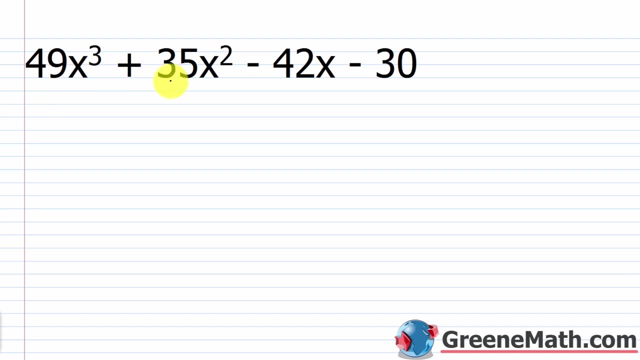 binomial, And that's what I have here. So either way you do that, you end up with the same answer. So a lot of different ways to kind of rearrange things and make things work. Let's take a look at another one Now. let's suppose we had 49x cubed plus 35x squared, minus 42x minus. 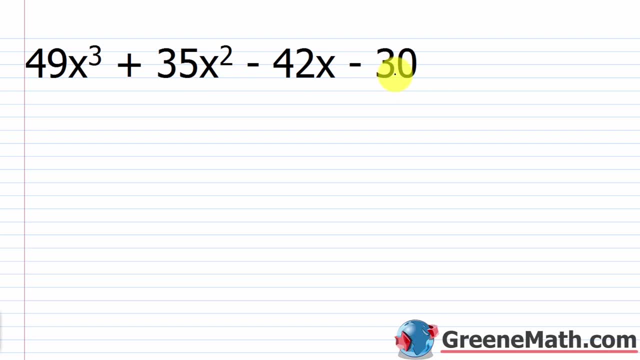 30. So again, the first thing I want to think about: is there anything that's common to everything I know? 49 is 7 times 7.. So again, Again, 7 is a prime number. so I go through and look at everything. 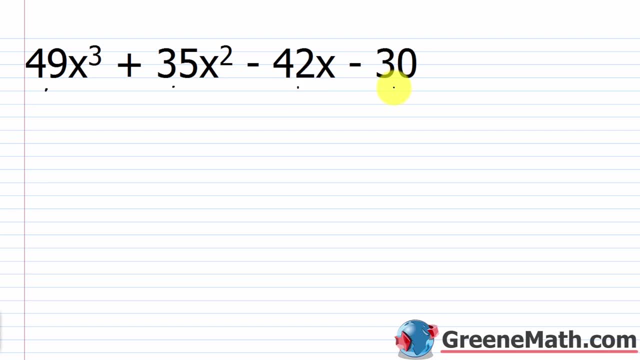 35 is divisible by 7,, 42 is divisible by 7,, but 30 is not, So I can't pull anything out. number-wise, Variable-wise it's the same. I've got x, x, x, but no x here. 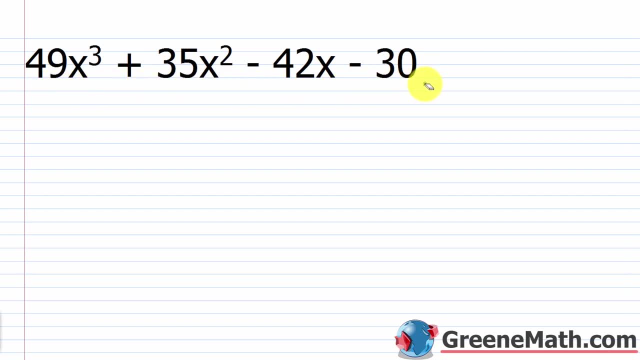 So I'm not going to be able to pull anything out other than a 1 or a negative 1, which again, it's a waste of time at this point. So now I would think about: okay, I want two groups of two terms each. 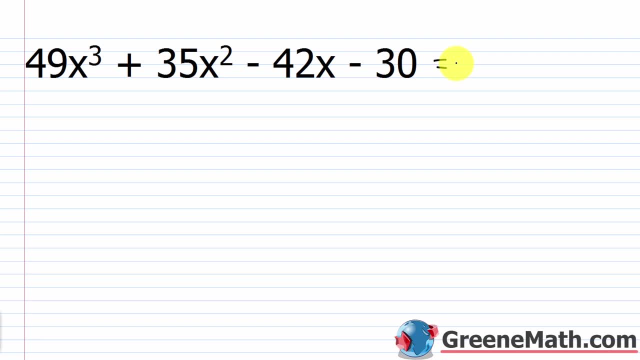 where each group has a common factor. Now again, that common factor might have to be 1 or negative 1.. So I would start by thinking about: okay, if this was a group, let's say this was group 1, what could I pull out? 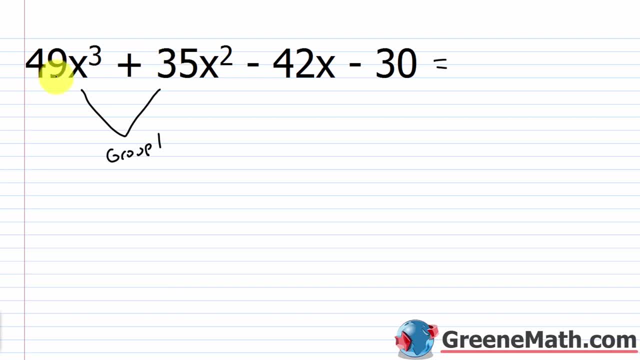 Let's just say I pulled out a 7, because both of these are divisible by 7, and then an x squared right. They each have an x. The smallest exponent is a 2. So 7x squared. What would that leave me with? 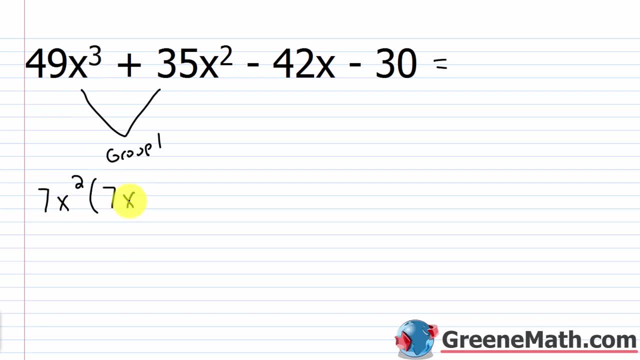 49 divided by 7 is 7.. x cubed divided by x squared is x. And plus 35 divided by 7 is 5.. x squared divided by x squared is 1.. So let's think about group 2 now. 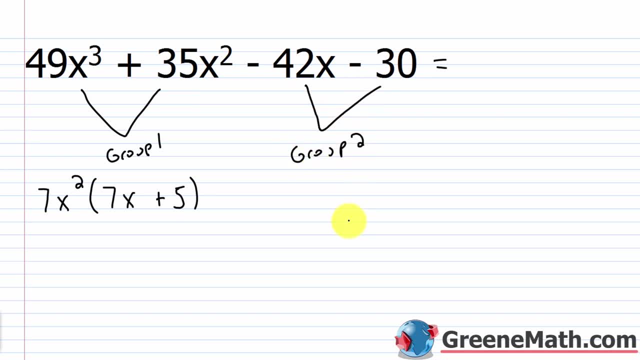 So this is going to be group 2. And our goal is to pull something out to where we end up with a 7x plus 5, that quantity. So what could we do? Well, we think about what's common. The first thing is, if I have 42 and I have 30,, 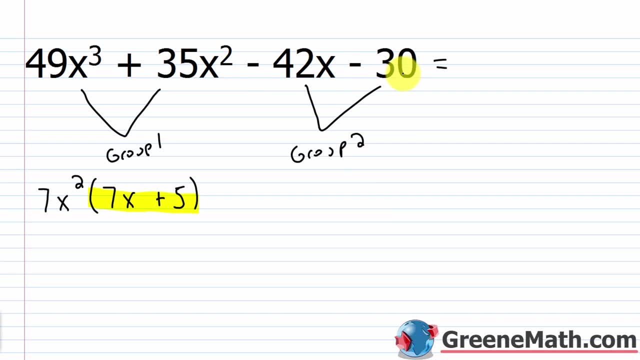 number-wise, the greatest common factor is a 6, right, Because 42 divided by 6 is 7.. That's a prime number. 30 divided by 6 is 5.. That's a prime number. So the best I could do is pull out a 6.. 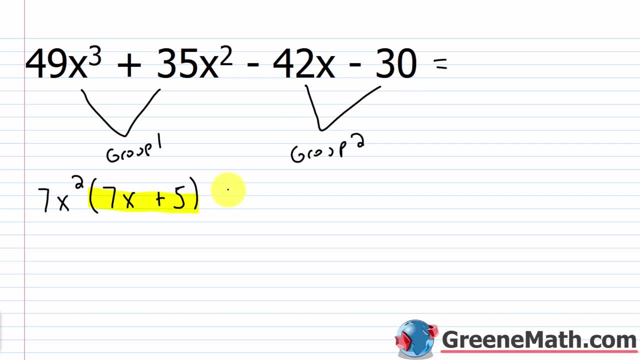 Now one thing you want to notice is if I pulled out a positive 6, the two terms inside the parentheses would be negative. The two terms inside the parentheses here are positive. So I could just do the opposite of that, Just pull out a negative 6.. 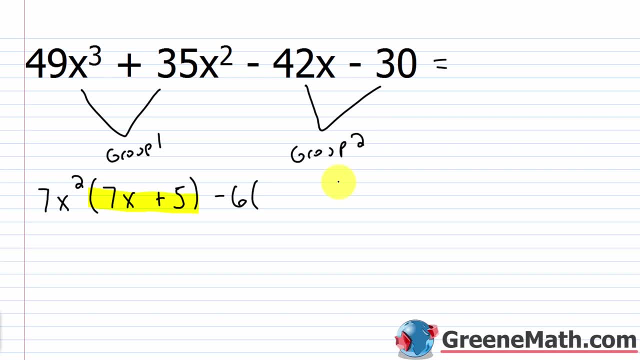 And what's going to happen is the two terms inside the parentheses would be: positive- Negative. 42x divided by negative, 6 would be positive: 7x Negative. 42x divided by negative, 6 would be positive: 7x- Negative. 30 divided by negative: 6 would be positive: 5.. 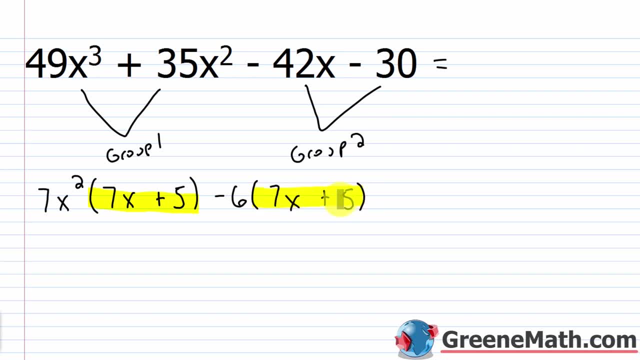 And voila, I get my common binomial factor of 7x plus 5.. So now I just want to pull that out Again. just pull that out. If I have the quantity 7x plus 5 outside, and then inside the parentheses, what's left? 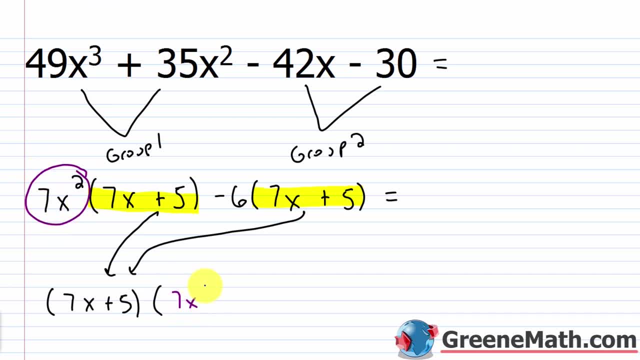 Okay, you think about what's left. We'd have a 7x squared and then you'd have a minus 6. Minus 6., Minus 6.. So let's get rid of the 7x squared, and this factors into the quantity 7x plus 5 times. 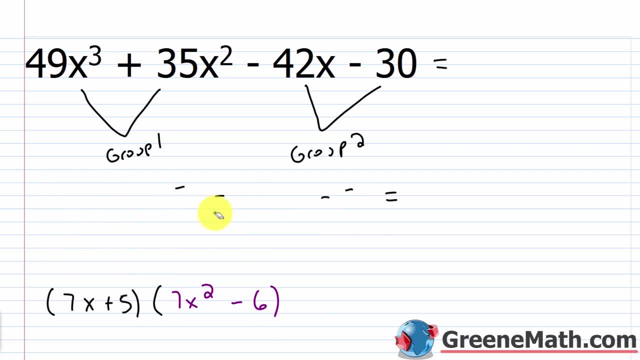 the quantity 7x squared minus 6.. And again, this isn't the only way you could have done that. I could have rearranged this into two different groups and gotten the same result. So let's say I did 49x cubed and then minus 42x. 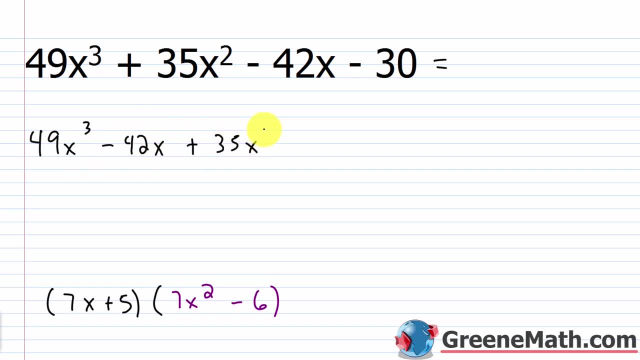 That's a group. Each would be divisible by 7x. And let's say I did another group. Okay, each is divisible by 5.. So in the first group I would pull out a 7x and I'd have 7x squared. 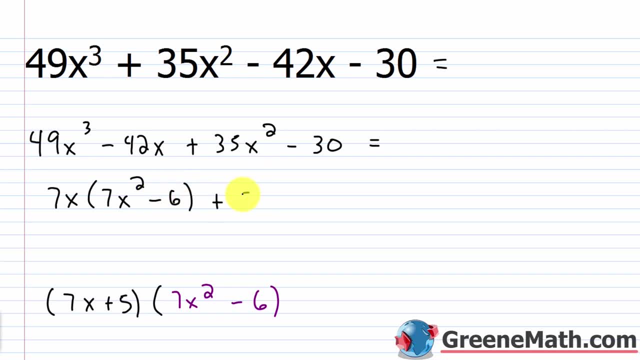 minus 6.. In the second group, I'd pull out a 5, and I'd have 7x squared minus 6.. So what do I get? Again, I have that common binomial factor of 7x squared minus 6,, which matches this. 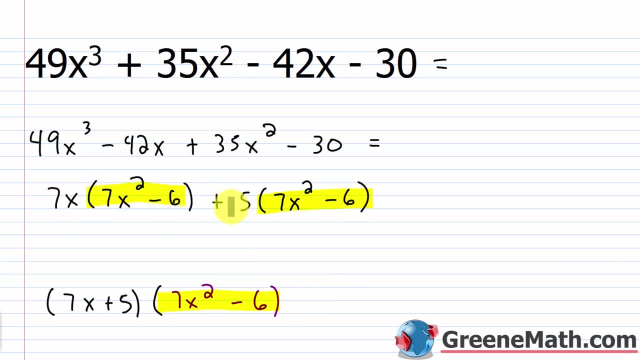 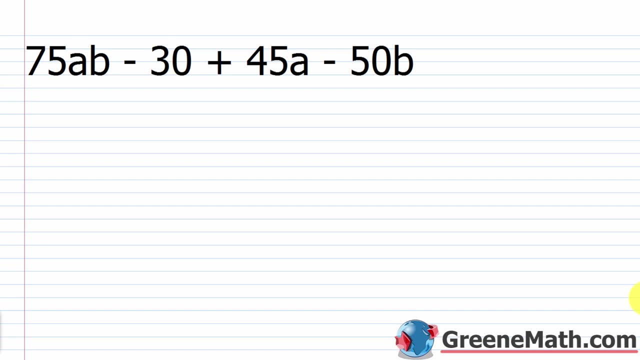 And then, if I pulled that out, I'd have a 7x plus 5, which matches this. So again, I'm just showing you. in a lot of cases there's more than one configuration that's going to work. All right, let's take a look at another one. So suppose we have 75ab minus 30 plus 45a minus 50b. 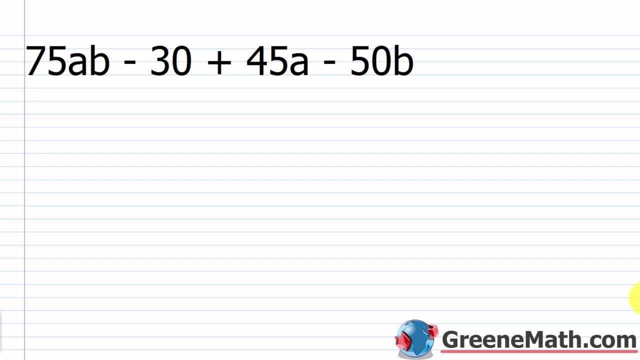 So the first thing again: is there anything I can pull out before I get started? Well, in this case there's going to be. Every number here involved ends in a 5 or a 0. So I know everything's divisible by 5, so I could pull that out. So if I pull out a 5 to start, 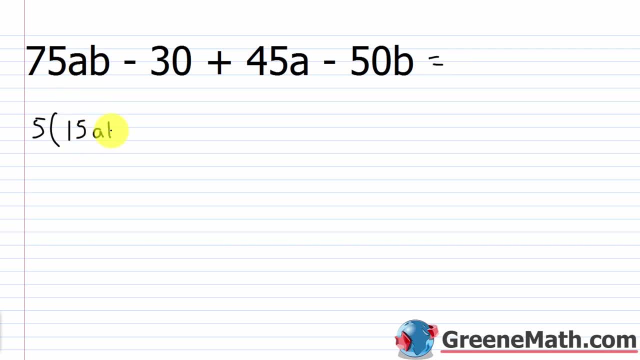 75 divided by 5 is 15.. So this would be 15ab minus 30 divided by 5 is 6, plus 45a divided by 5 would be 9a minus 50 divided by 5 would be 10, then times b would be 10b. So we pull that out before. 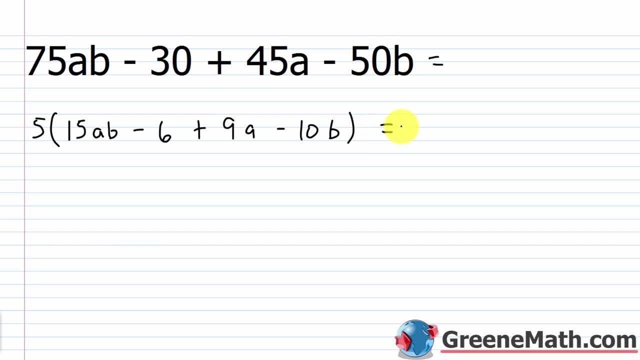 we even begin Continuing. I do my normal process with the inside part. Forget about the inside part. I'm going to do the inside part. I'm going to do the inside part. Forget about the 5 outside. That's just going to multiply, whatever the result of this is. 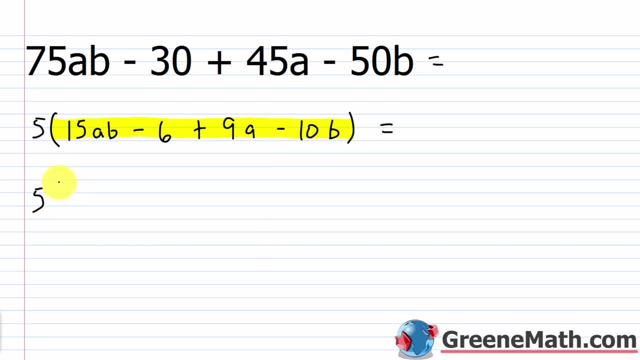 So inside here let me just write the 5 again. I'm looking for two groups of 2, where each group has a common factor, And again that common factor might end up being 1 or negative 1.. Now, one thing that you would see right away if I look at 15ab and I look at 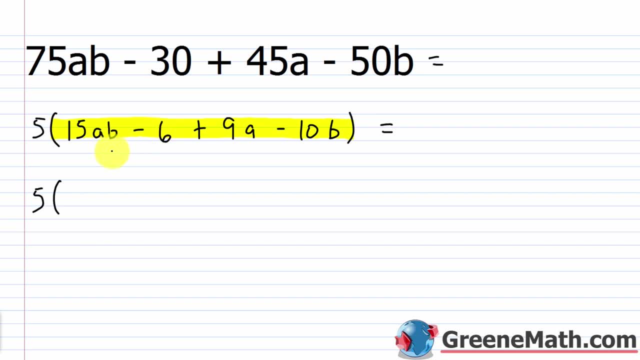 negative 6, they don't share a b. okay, Only a b in this term. If I look at 9a and negative 10b, again they don't share a b. I'm going to want to put the terms with bs next to each other. Let me show you what happens if I don't. So: 15ab minus 6 plus 9a. 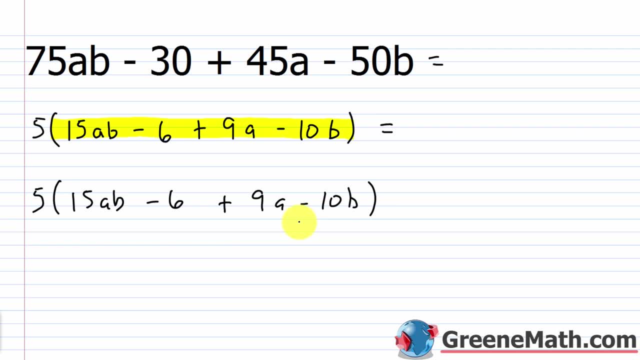 minus 10b. There's no way to factor this the way it is. If I look at this group of 2, I could pull out a 3, okay, I could pull out a 3. And what would be left is 5ab. 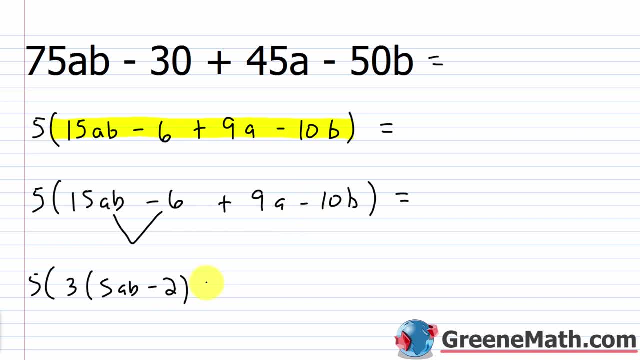 Minus 2. But over here I can't pull out anything. So plus I could pull out a 1 if I want or a negative 1.. Let's just try 1.. So 9a minus 10b. I don't have a common binomial factor here. 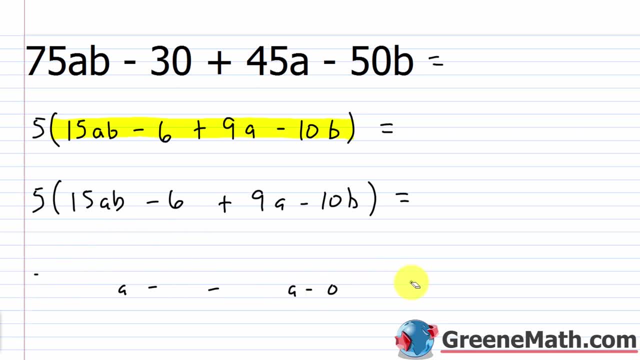 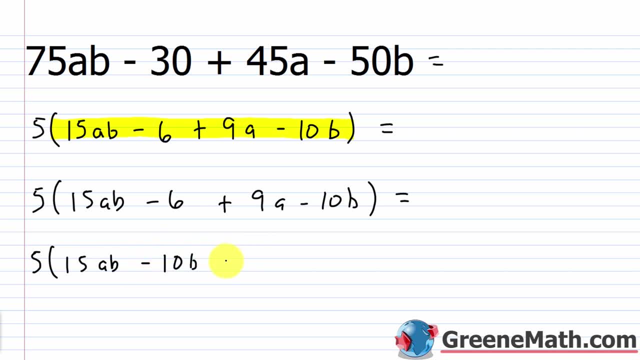 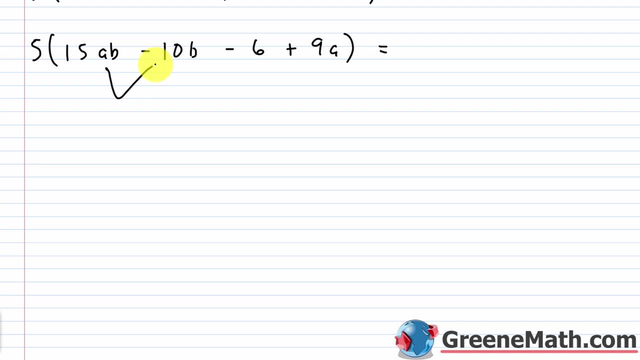 get some room going. If I look at this first group, what can I pull out? Well, I can pull out a 5b. So 5 times I pull out a 5b from there And inside of the parentheses, 15 divided by 5 is: 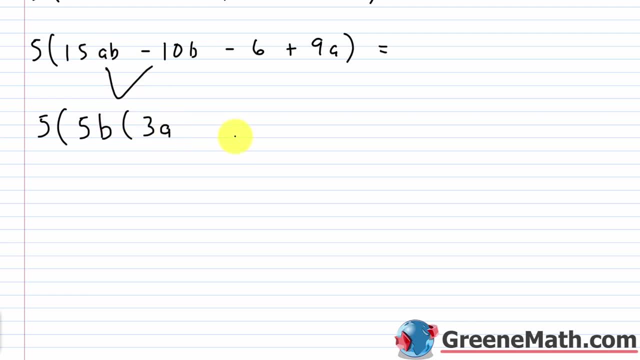 3. ab divided by b would just be a. Then if I did negative 10b divided by 5b, I'd have minus 2.. Now from this next group I can pull out a positive 3 or negative 3.. Let's just start. 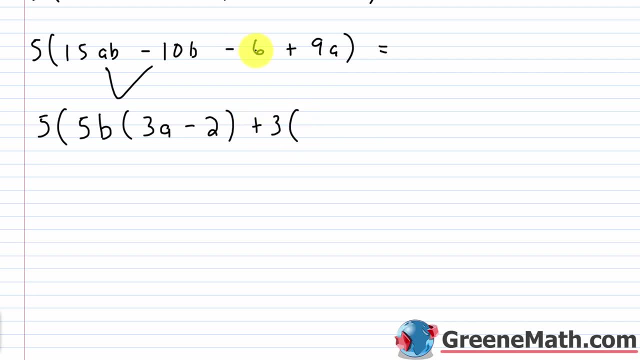 by pulling out a positive 3.. So if I pulled out a 3, I'd have negative 6 divided by 3, which is negative 2.. Then 9a divided by 3 would be plus 3a. Now, a lot of you at this. 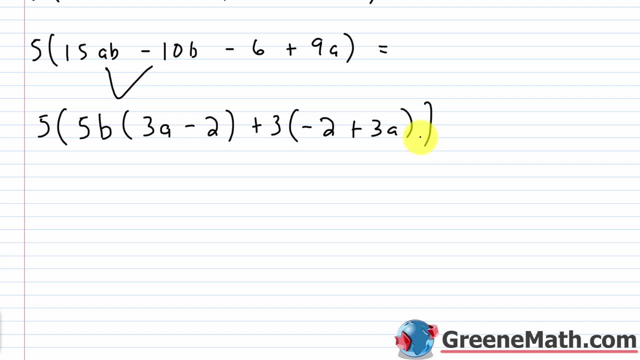 point. if you came to this would say: oh, I don't have a common binomial factor. But pay close attention. here You have 3a minus 2, and you have negative 2 plus 3a. Those are the same. Remember, if I'm adding, I can switch the order. If I just switch the order here, okay, 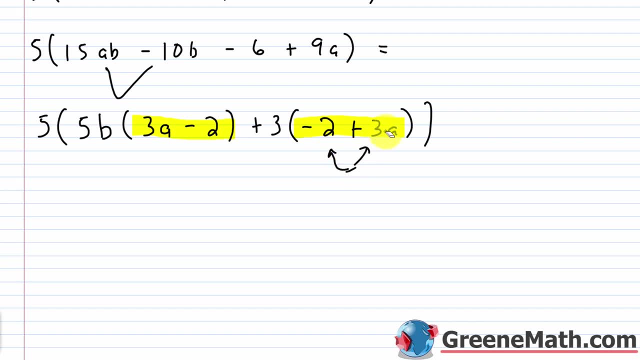 and just change the terms around, I've got the same thing, So I can just put 3a minus 2.. 3a minus 2 and now I have a common binomial factor. So if I factor that out, remember, the five stays out in. 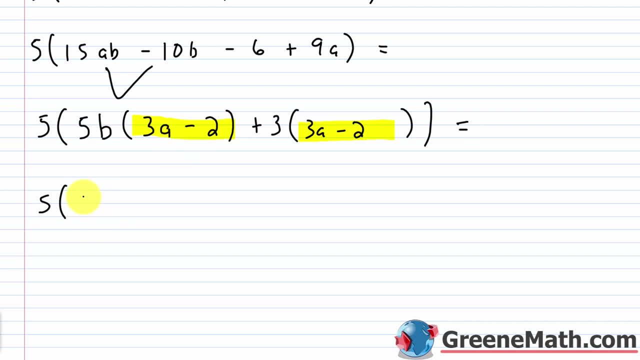 front, I would have 3a minus 2.. 3a minus 2 times again. if I pulled this out, what's left? Well, I have 5b plus 3.. So 5 times the quantity 3a minus 2 times the quantity 5b plus 3.. And again there. 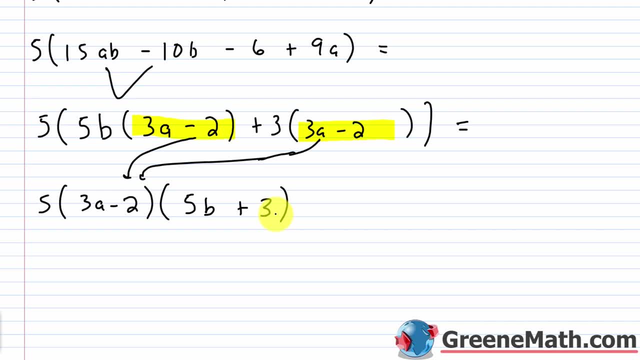 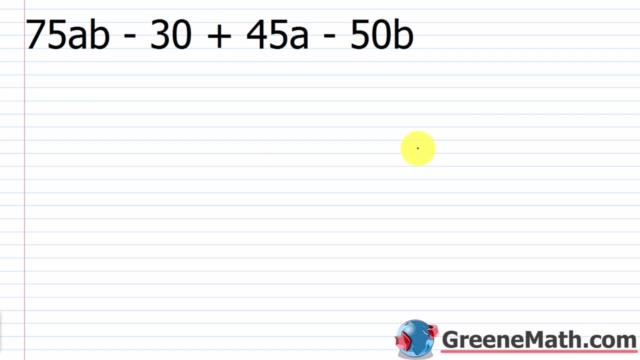 are scenarios where you have to change things around, otherwise it will not work, and that's a perfect example. So I just wanted to quickly come back up to the original problem and I want to show you what happens if I don't pull a 5 out to start, If I don't pull a 5 out to start. we already know. 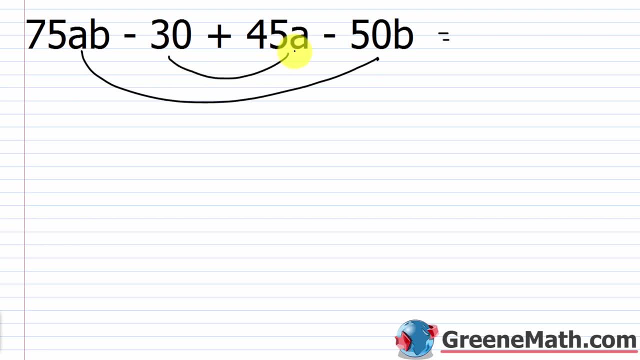 that I can put these two next to each other and these two next to each other and I will get a common binomial factor. So let's do that, Let's do 75ab minus 50b and then let's switch the order here and just put plus 45a minus 30.. So, from the first group, if I think about 75 and I think about 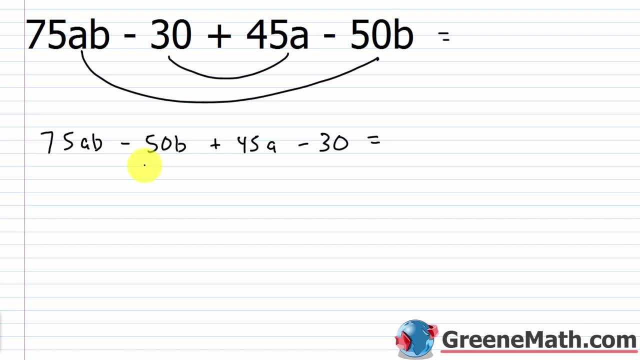 50. I know that the GCF is 25.. So 25. and then I know that I have a b here and a b here, So let's do 25b. So 75 divided by 25 is 3.. ab divided by b is a. Then minus 50 divided by 25 is 2.. b over b is 1.. 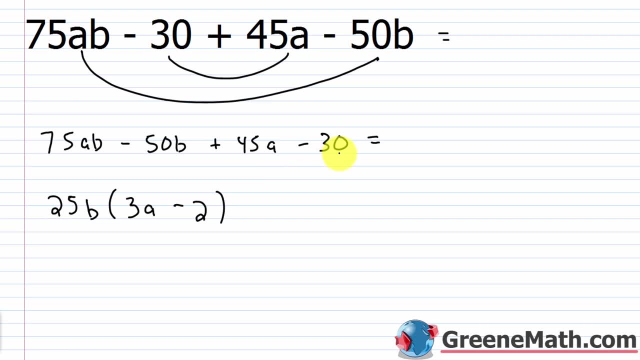 So from these two, 45 and 30, I know that I could pull out a 15.. So if I pull out a 15, I would have 45 divided by 15, which is 25b, Which is 3. Then, times a, and then negative, 30 divided by 15 is negative 2.. So let's continue. 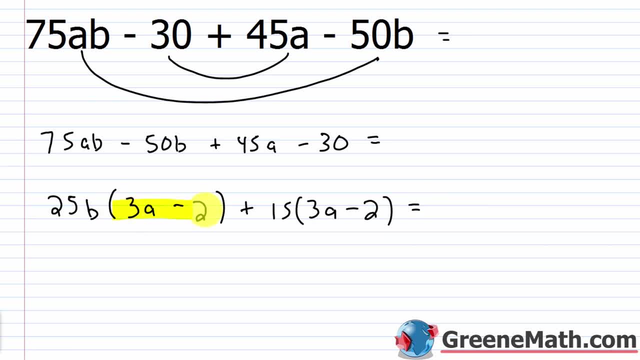 here I've got a common binomial factor of 3a minus 2.. All right, so that would come outside. So 3a minus 2, and then what's left when I pull that out? Well, I'd have 25b plus I'd have 15.. Now you, 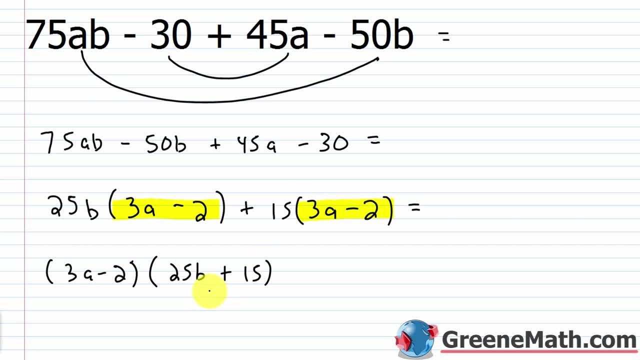 might say: well, okay, that's fine, It's not. Whenever you factor, you must factor completely Okay. so is there anything that you can do to make sure that you have a common binomial factor of 3a minus 2?? Is there anything else that I could pull out from 3a minus 2?? No, there isn't. Is there anything else I could pull out from 25b plus 15?? Yes, there is. 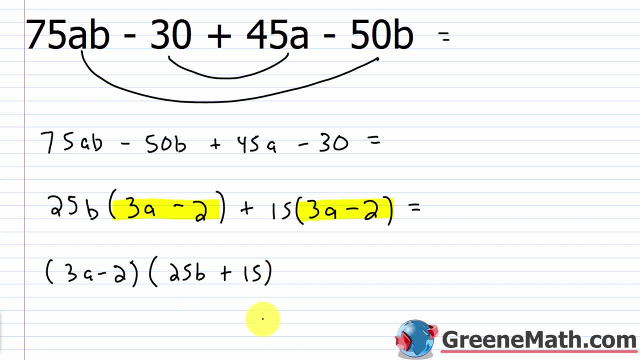 25 is divisible by 5, and so is 15.. So I would actually have to pull a five out from this and say that–and I'm just gonna switch the order to make this convenient–I'd have 5 times–25 divided by 5 would be 5–then times b–plus 15 divided by 5 is 3–then times this other couple. 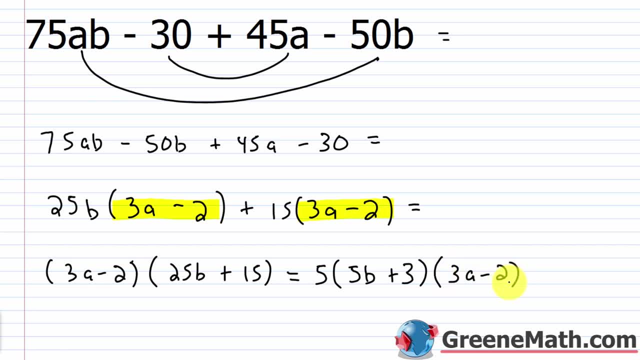 3a minus 2.. So if I reported this as my answer, which is a common mistake, I'm not going to get full credit because I didn't factor completely. When I look at this answer, 5 times the quantity 5b plus 3 times the quantity 3a minus 2, I've factored completely. Nothing else I can take out. 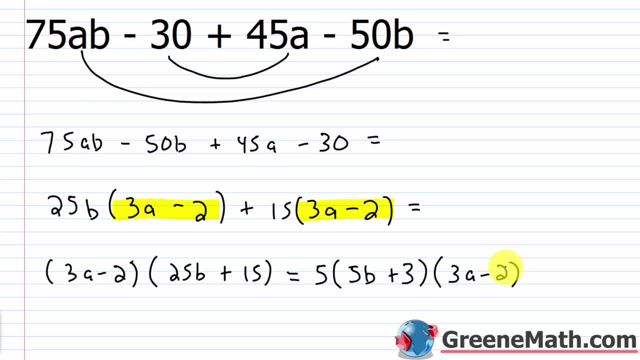 of here. Nothing else I can take out of here right Other than 1 or negative 1.. And again, that's why I preach to pull something out if it's common when you begin, because then you don't have to worry about this happening at the very end. So let's look at one more, and we're just going. 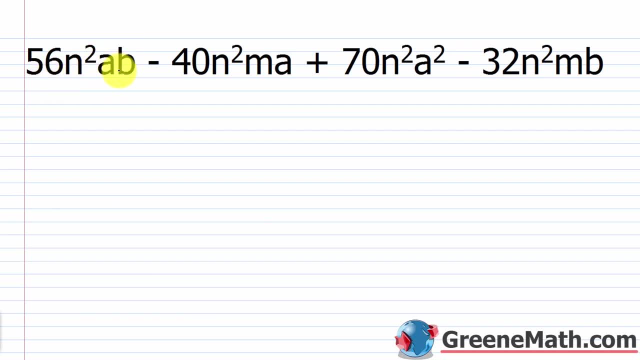 to wrap this lesson up. So we have 56n squared ab minus 40n squared ma, plus 70n squared a squared minus 32n squared mb. So let's see if we can pull anything out. 56, I know, is 8 times 7.. 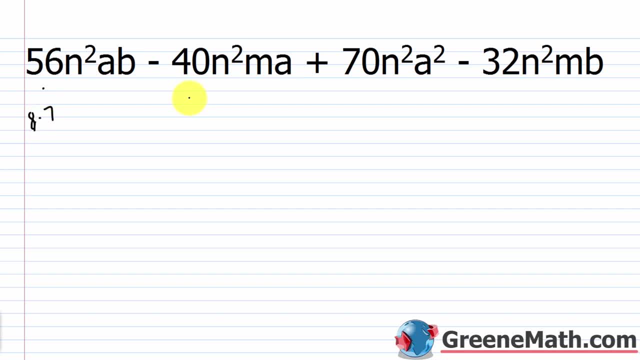 And I know 8 is too cute, but let's not go that far. 40 is 8 times 5.. 70., I would think about 10 times 7.. And 32 would be what 8 times 4.. Now forget about the 7 and the. 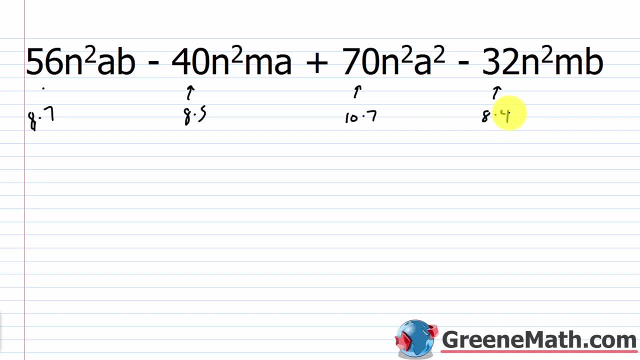 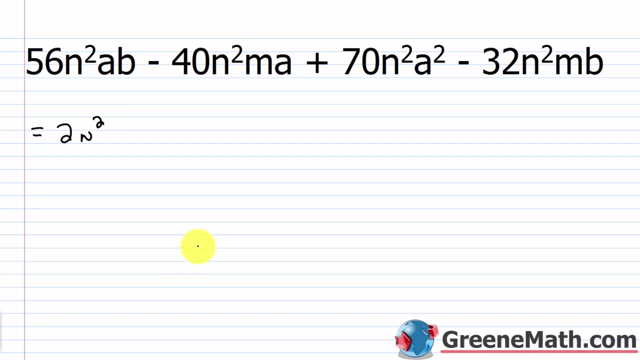 pull that out. Then I think about a. So I have an a here, an a here and an a here, and an a here, but not an a here. Then I think about b: A b here, but not here. Then I think about m. 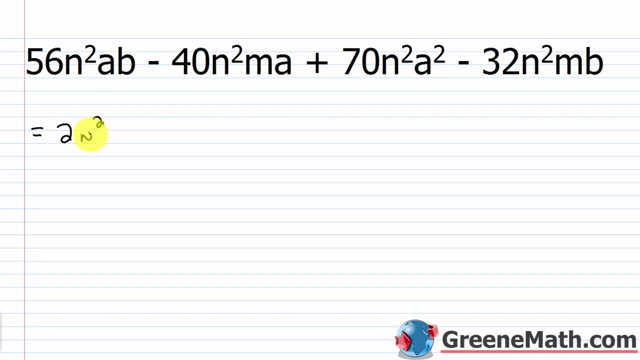 and there's no m here. So really all I can pull out is 2n squared. That's fine. So, inside of parentheses, 56 divided by 2 would be 28.. n squared over n squared is 1.. So I just have 28ab. 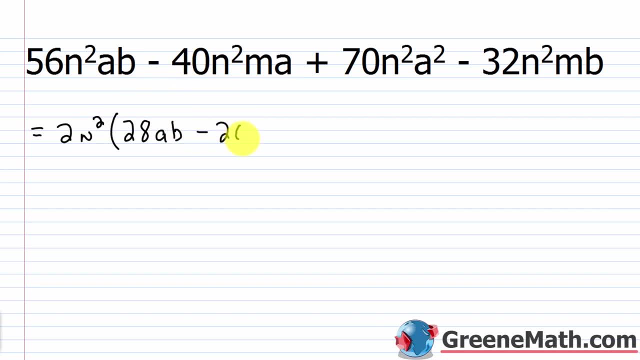 Then we have minus. You think about 40 divided by 2.. That's 20.. n squared over n squared is 1.. And then you'd have ma, or you could write: am Doesn't matter. Plus 70 divided by 2 is 35.. n squared over n squared is 1.. And then a squared. 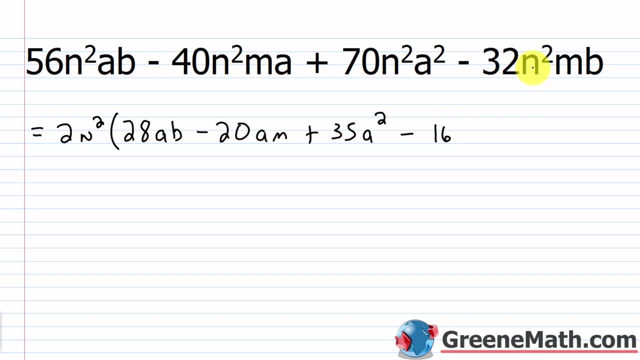 Then minus 32, divided by 2, is 16.. n squared over n squared is 1.. So you'd have mb or you could put bm Okay. So let's think about if we had a group here and a group here, Would that work out? 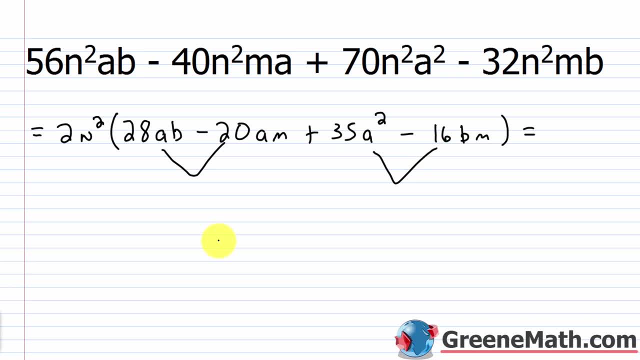 Well, I just think about the variables for a minute. If I look at this one right here, I pull out an a, I would have a b and an m. I can't pull any variables out here, so I'd be left with a squared. 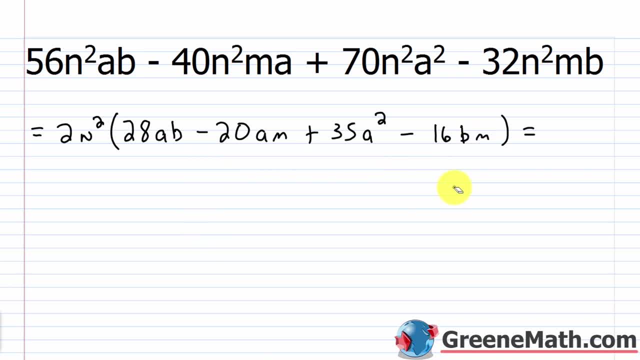 and bm. So that configuration is not going to work. I don't need to waste my time. So, configuration wise, what I want to think about is putting these two next to each other because they each have an m. So I'd be left with an a and a b. I pulled out the m With these two. they each have an a. 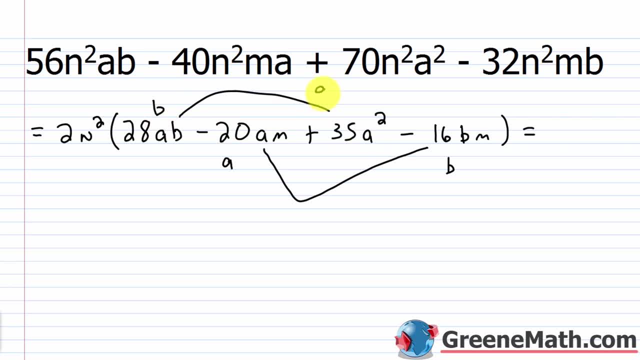 so if I pulled out the a, I'd be left with a b and I'd be left with an a. So that's what I want. You can see that that would work out. Might have to change the order around, but again, if you're adding things that doesn't matter, All right. So I want to flip the. 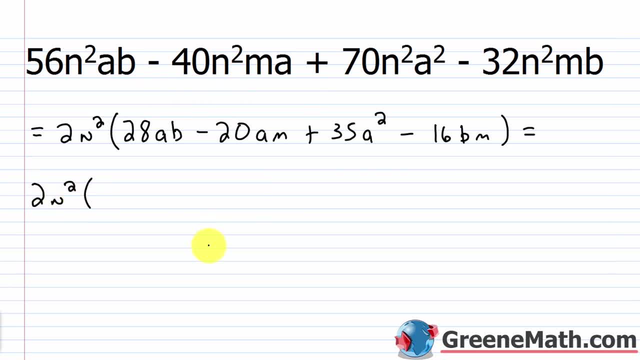 configuration. Let's do 2n squared, Let's take 28ab and let's stick that next to plus 35a squared And just for the sake of completeness let's go ahead and just rearrange that. Let's say we have 35a squared plus 28ab. Let's do it that way. 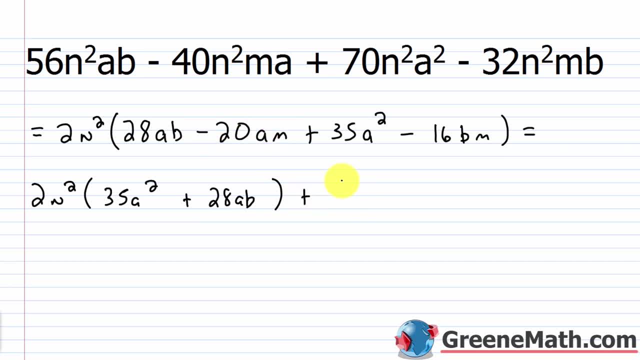 Okay, Minus 20am. So let's put plus- I'm just going to put this in parentheses- negative 20am And then minus you have this 16bm. So from the first group I'm just going to copy: 2n squared: 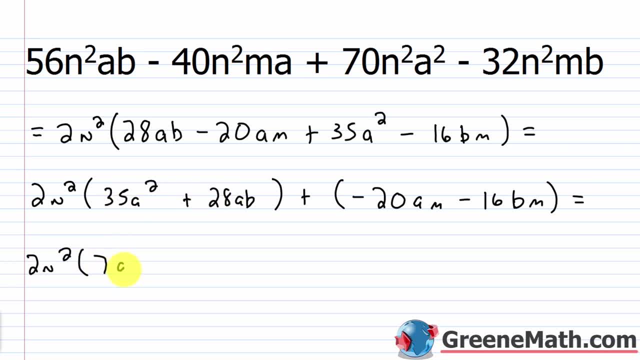 So from the first group here I could pull out a: 7a. What's left? 35 divided by 7 is 5.. a squared over a is a, Then plus 28 divided by 7 is 4.. ab over a is b, Then plus. 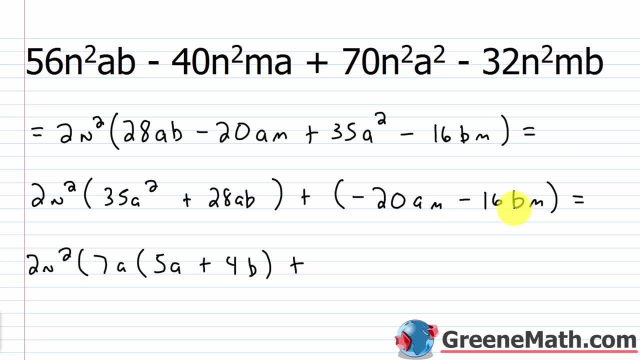 you have this 16bm, So from the second group I can pull out a negative, because both of these are positive. So let's do negative. And then 20 and 16 are each divisible by 4. So let's do. 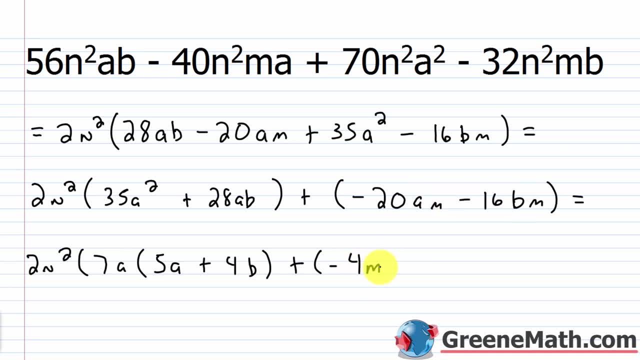 negative 4.. And then there's an m that's common, So negative 4m. So inside I'd have negative 20 divided by negative 4, which is 5.. am over m, which would be a, Then negative 16bm divided by. 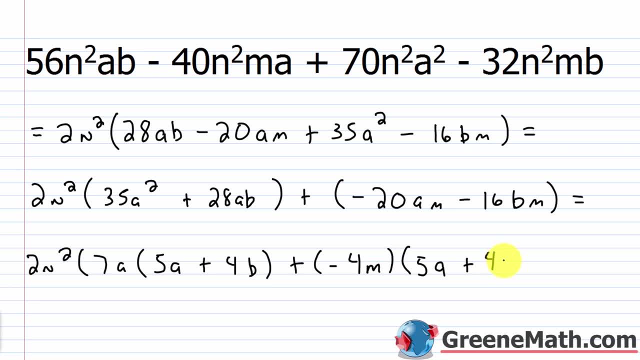 negative 4m is positive 4b. So what do I have here? I have a common binomial factor of 5a plus 4b, So this will be 2n squared times. if I pulled this out, I'd have that 5a plus 4b. And then what's left? Well, I'd have 7a. 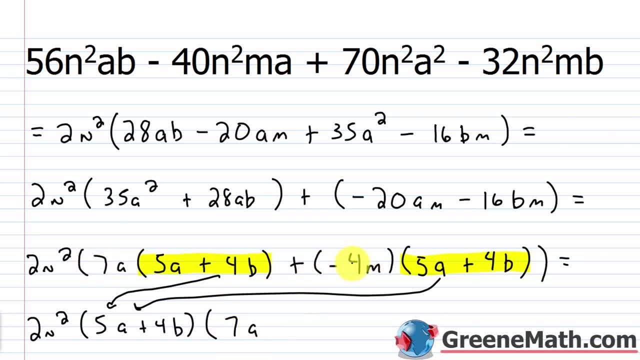 plus over here I would have negative 4m. So I'm just going to write minus 4m. So we end up with 2n squared times the quantity 5a plus 4b, times the quantity 7a minus 4m. 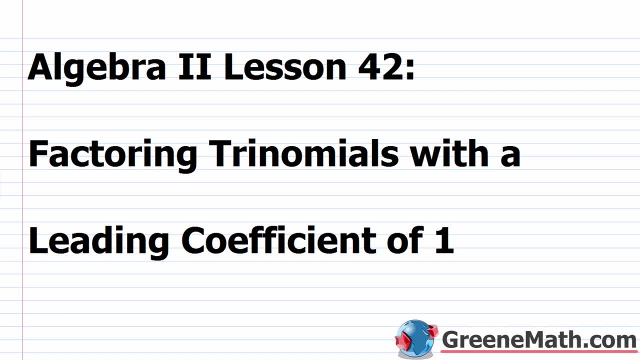 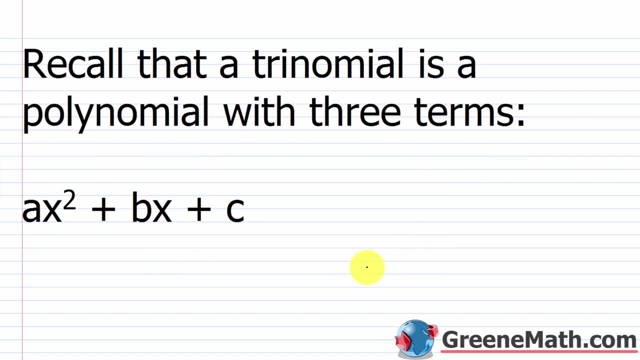 Hello and welcome to Algebra 2, Lesson 42. In this video, we're going to learn about factoring trinomials with a leading coefficient of 1.. So once again, we're on a topic that, if you took an Algebra 1 course, you're very familiar with this. This is a very, very easy scenario to deal with. I 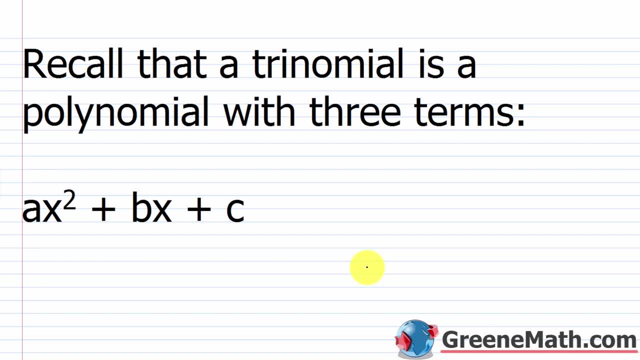 just want to start by talking about what a trinomial is and how we're going to factor it into the product of two binomials. So I want you to read this: It's going to be a group of three trinomial, So a trinomial is a polynomial with three terms. 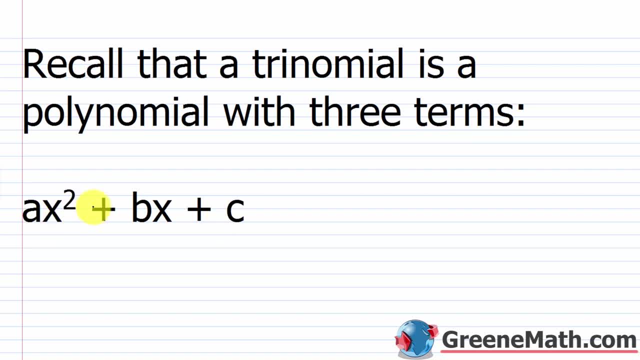 So, as a generic example, this is a trinomial. We have ax squared plus bx plus c, So you've got a term, a term and a term, Three terms. that gives you a trinomial. Now, in this particular, 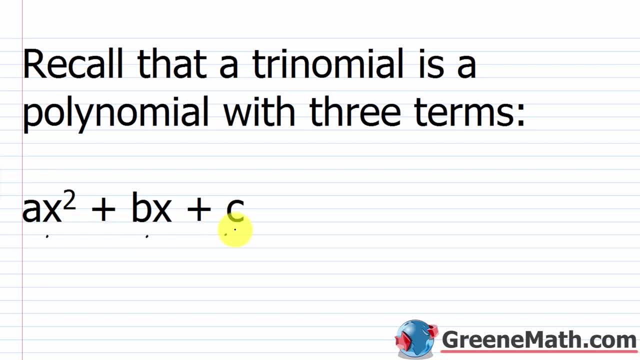 case that we're going to look at today. we're going to factor this trinomial where the leading coefficient- in this case that's represented with a- is going to be a 1, and it's going to be factored into the product of two binomials, or the number of binomials And the number. 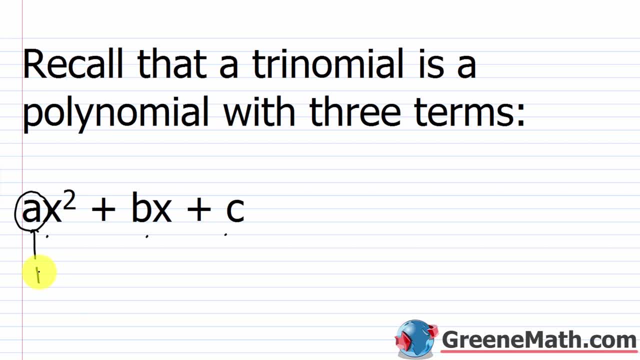 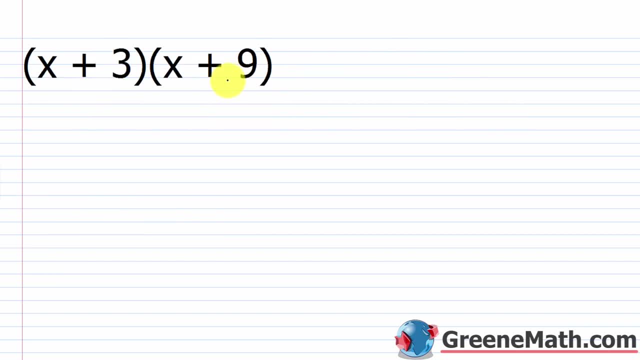 of binomials that you get when you have a trinomial equals something like 3.. So I want to start two binomials, okay. So one binomial times, another binomial. Now, when we have a binomial times, another binomial, we already know a shortcut for that, known as FOIL. okay, So if I just use FOIL, 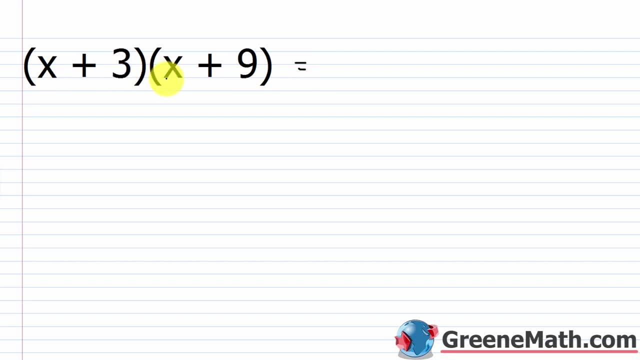 here. let's just observe a few things You do first times. first, x times x: is x squared. Then the next thing I would do is: the outer x times 9 is plus 9x. Then the next thing I would do is the inner 3 times x is plus 3x. Then the last thing I would do is the last 3 times 9 is. 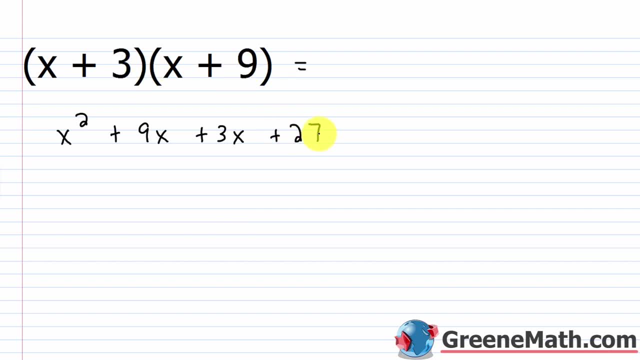 plus 27.. Now if I have x squared plus 9x plus 3x plus 27,, I can combine like terms and I can say this is x squared plus 9 plus 3 is 12.. So the middle would be 12, and then that common variable. 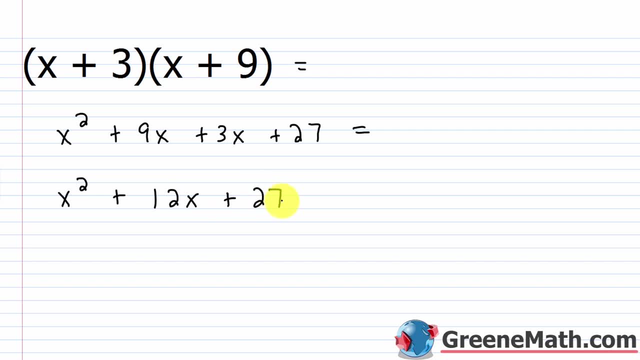 of x and then plus 27.. So the question for today is: how do we solve this problem of x squared plus 9x plus 27?? Let's go from this to this. okay, We're going to be factoring, Remember, that's the reverse. 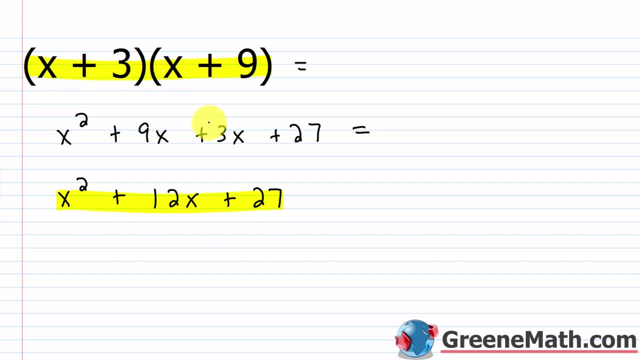 of the distributive property, which is what FOIL really is. So if I'm going to go from this to this, let's just do it in reverse. I know that I would set up two sets of parentheses here, And if the leading coefficient on this is a 1,, well then, I know that this times this. 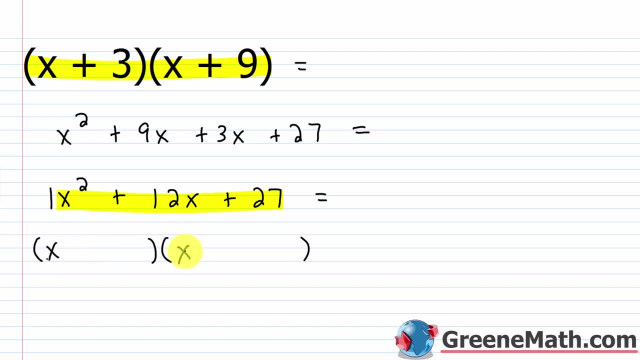 gives me this. So this is going to be x and this is going to be x squared, So that's always going to be the case. If I had y squared in this position, this would be y, and this would be y. If I had z squared z and z. If I had q squared q and q. 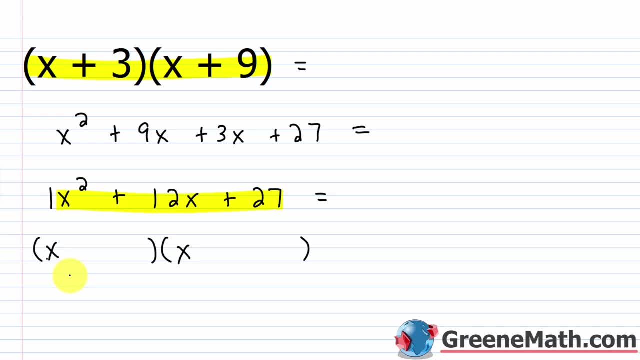 Okay, so the first position of each is very easy to get. Where you have to think a little bit is there's four steps to FOIL, So you need the o, the i and the l. You've got to work that out. 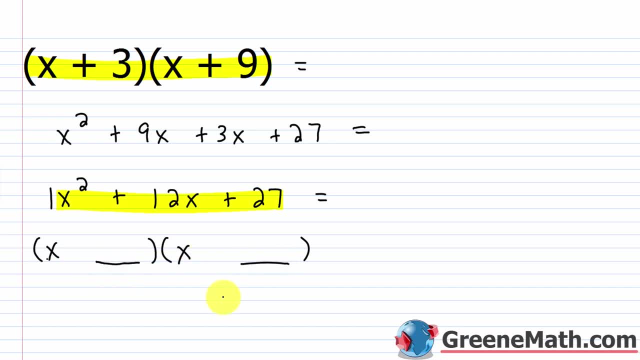 And the way you work that out is you need two integers here that are going to sum to this middle coefficient, the coefficient for x to the first power, And that's going to give you a product of this final constant term. So you would say you want. 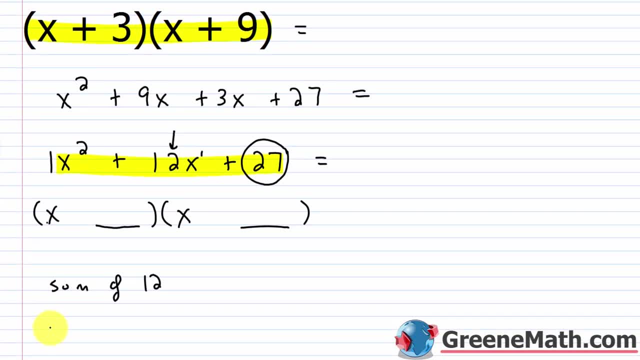 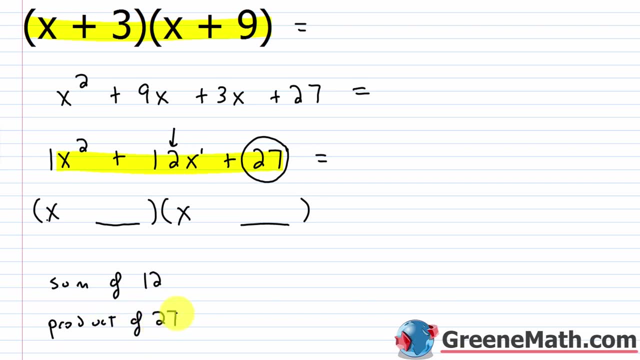 a sum of 12 and a product of 27.. And why is that the case? Well, the outer and the inner. if you remember this step, the outer was 9x, the inner was 3x. We add those together. 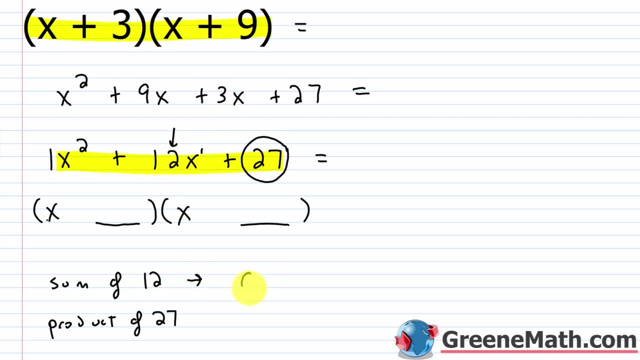 that gives us 12x. This we're looking from the outer plus the inner, And then this comes from the last 3x9, that gave us 27.. So we're working out these three by just finding out two integers. 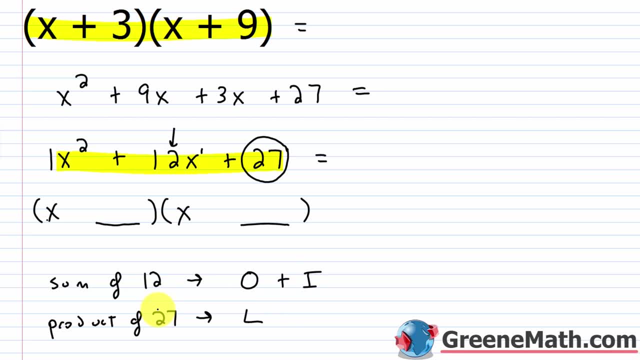 whose sum is 12 and whose product is 27.. And we can see that 9 and 3 gave us the 12 in the middle, and then 9 and 3 gave us the product of 27 in the end. So if I started without knowing this, 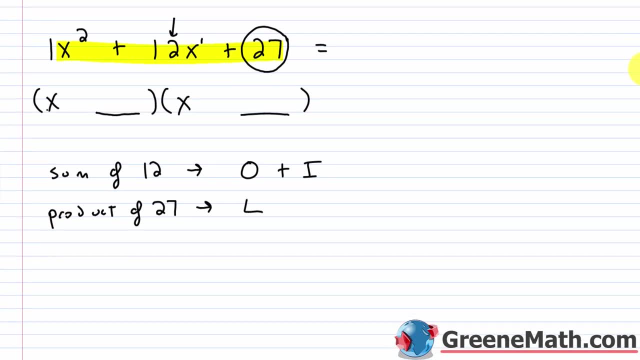 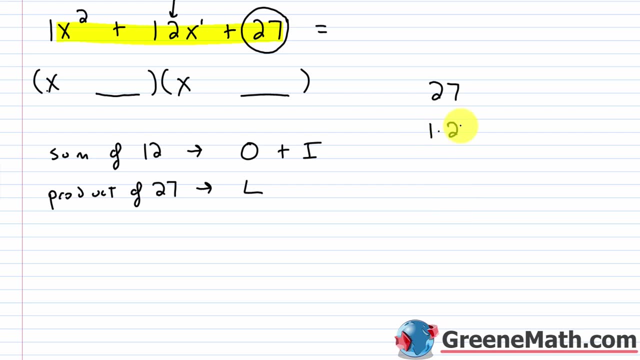 information. if I just scrolled past it and said this is what I have if I take 27,. really, the only factors would be what? 1 times 27 or 3 times? not. I can't really do anything else, So I'd have to work with 3 and 9, and that happens to work in. 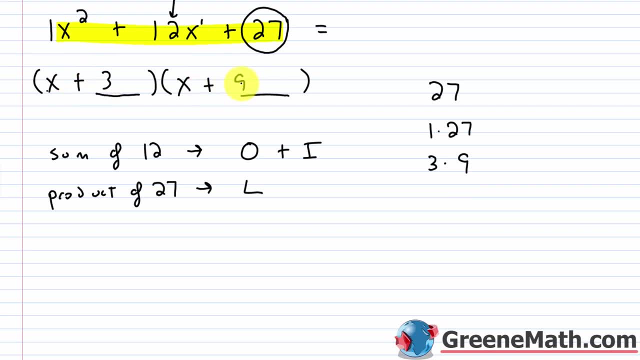 this case x plus 3, and then x plus 9.. So that's how you go back and forth. You just find two integers whose sum is the middle term and whose product is the final term. The first spot in each is going to be super simple. 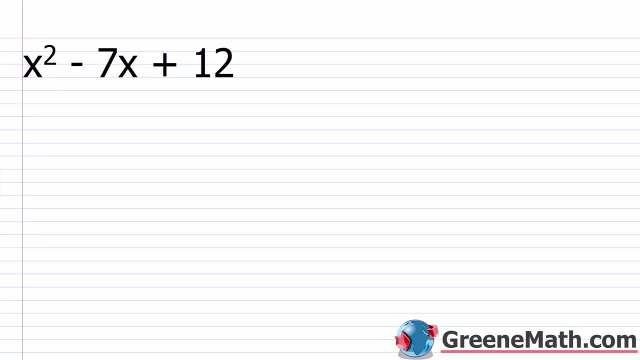 So you just have to work out the final spot in each. So let's take a look at an example, And if you didn't understand anything that I just said, that's okay, because you're going to pick this up right away. So the first thing that I tell people to do is just set up the parentheses, If you just 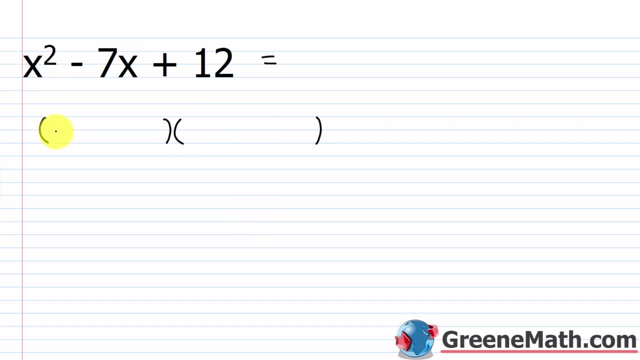 get that set up and say, okay, well, I know, if this is x squared for my first it would be x and then x. All I have to do now is fill in this blank and this blank- Very easy to do- Find two. 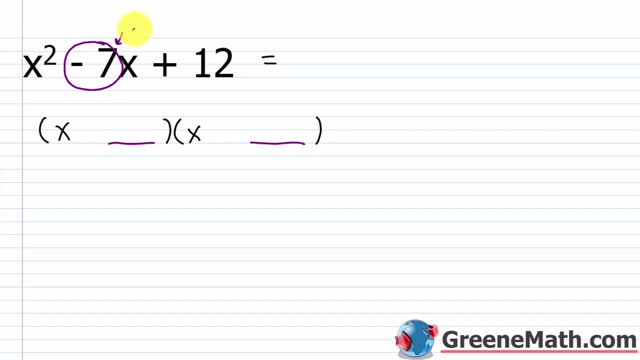 integers whose sum is 9 and 3.. And then I'm going to go back and forth. So I'm going to go back and forth, So I want a negative 7.. So I want this for the sum and whose product is 12.. So I want a. 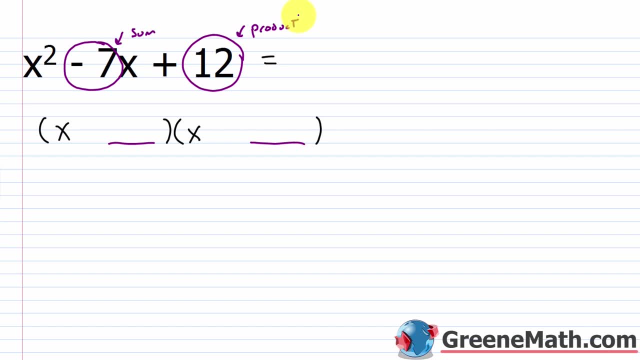 product of 12.. Now, if I think about 12,, if I factor it, I've got 1 times 12.. I've got 2 times 6.. I've got 3 times 4.. Now let me stop for a second, If I want a positive product but a negative sum. 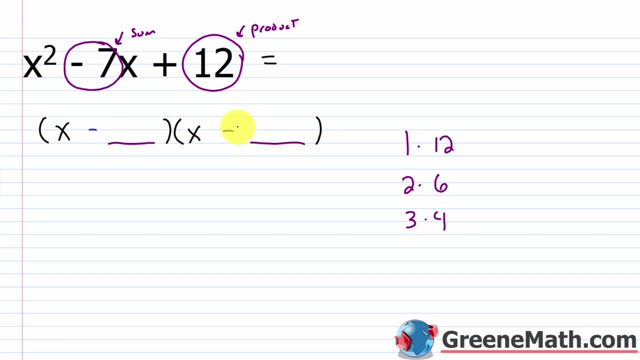 I know that I've got to have a negative and another negative. Negative times negative is negative plus negative is negative. So, thinking about my two integers, I know that negative 3 and negative 4 would work perfectly. Negative 3 times negative 4 would be positive 12.. Negative. 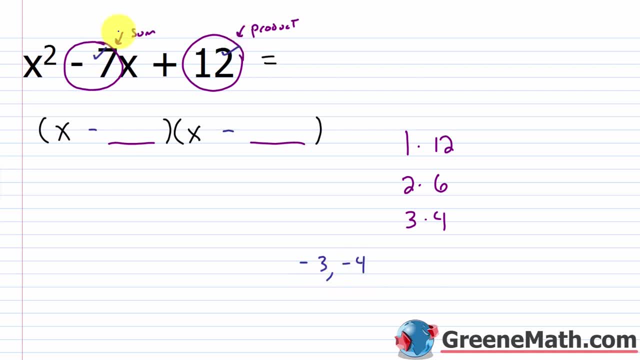 3 plus negative 4 would be negative 7.. So what I want here is x minus 3, that quantity times the quantity x minus 4.. And if you want to, you can check this with FOIL: x times x is x squared. 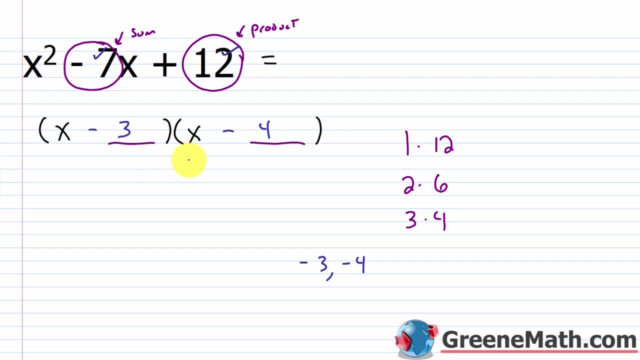 The outer would be minus 4x, the inner would be minus 3x. You sum those, you get negative 7x. And then the last would be negative 3 times negative 4,, which is 12. So you would get x. 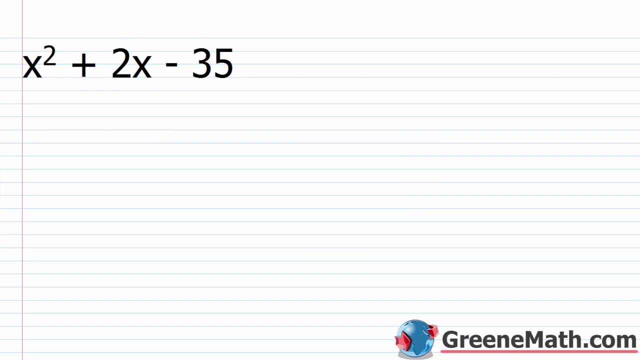 squared minus 7x plus 12 back. All right, so for the next one I'm going to look at it's x squared plus 2x minus 35.. So again, I want to set up my parentheses here. I don't want to just say okay. 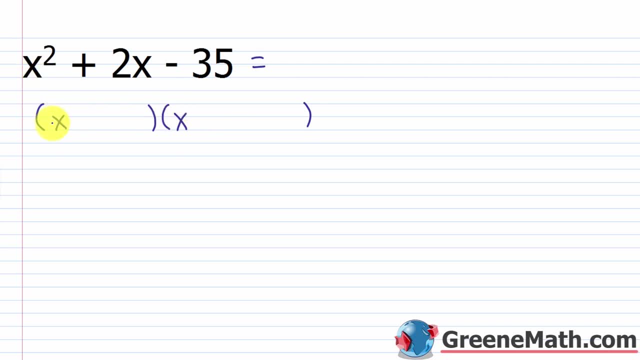 well, I know that this times this will give me this, So I need x and x. The first position in each one is always a breeze to get. It's this position here and here that we have to do a little work for Again. 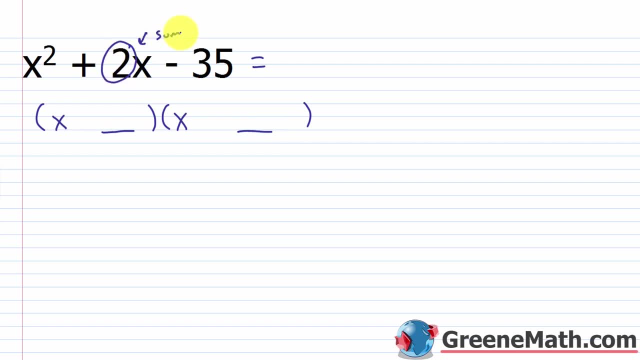 two integers that are going to sum to 2. So sum to the coefficient for that middle term, and then whose product is that constant at the end? So this is the product. All right, so two integers. We think about negative 35. If I have negative 35 as a product, 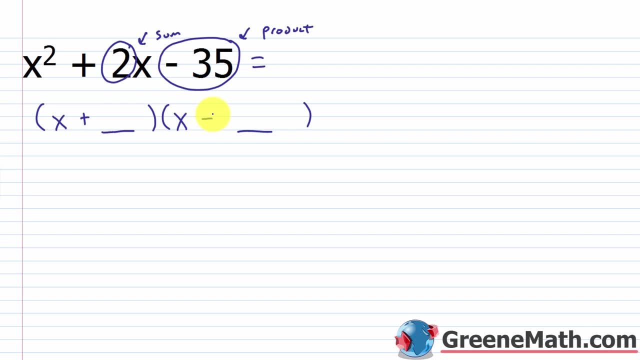 one of these has to be positive, one of these has to be negative. So just think about 35 for a second. You've got 1 times 35.. Can't play with the signs and make that work. It's not divisible by 2,. 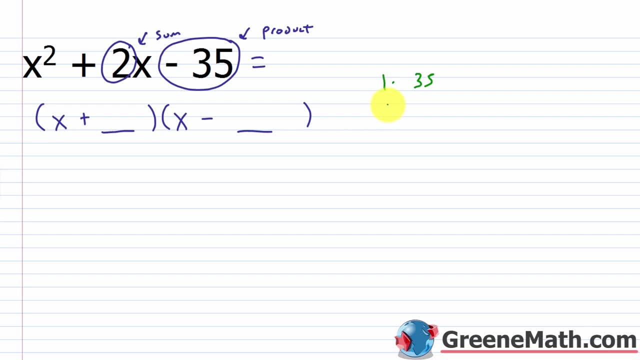 it's not divisible by 3.. Not divisible by 4,. it is divisible by 5.. I've got 5 times 7.. Now I can make 5 and 7 work, but I've got to play with the signs. The sum is positive: 2. So the larger absolute value needs to. 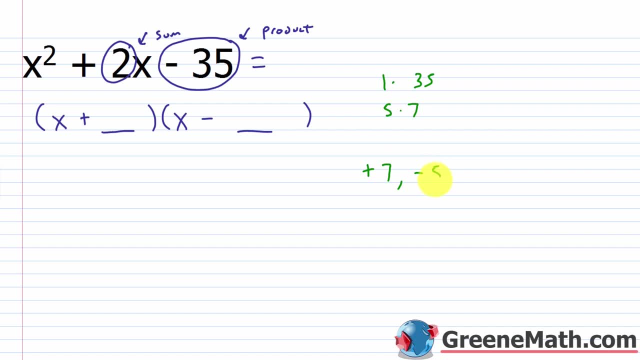 be positive. So if I do positive 7 and I do negative 5, that will work. Positive 7 plus negative 5 is going to give me positive 2.. Positive 7 times negative 5 is going to give me negative 35. So what I want is the quantity x plus 7, which is going to give me negative 35.. 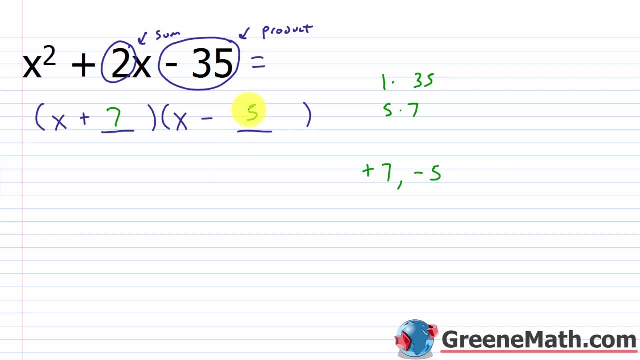 So what I want is the quantity x plus 7 times the quantity x minus 5.. Let's take a look at n squared plus 12n plus 20.. So again, let me just set up my parentheses here And again, if this is n. 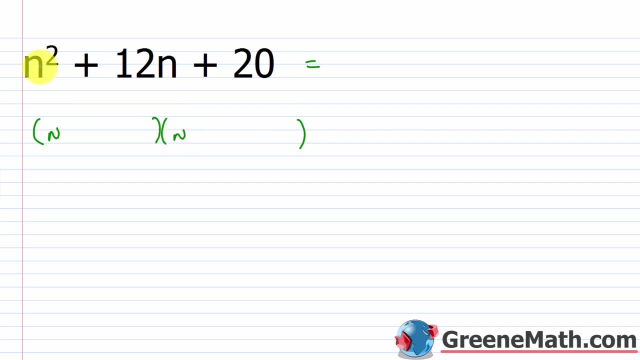 squared, then this is n and this is n. If it was q squared, this is q and this is q. So very easy to get the first position in each Again where we think is right here and right here, So two integers whose sum is 12.. Okay, the sum is 12.. And the sum is 12.. So, the sum is 12. And the sum is. 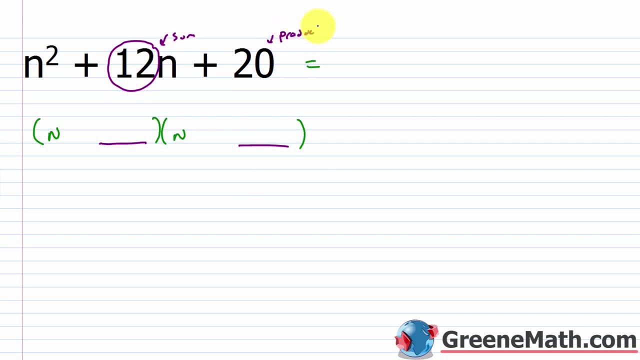 12. And the product is 20.. Now, if I think about factors of 20,, I think about what you have one times 20, that's not going to work. Two times 10, that would work. Two times 10 is 20.. Two plus 10. 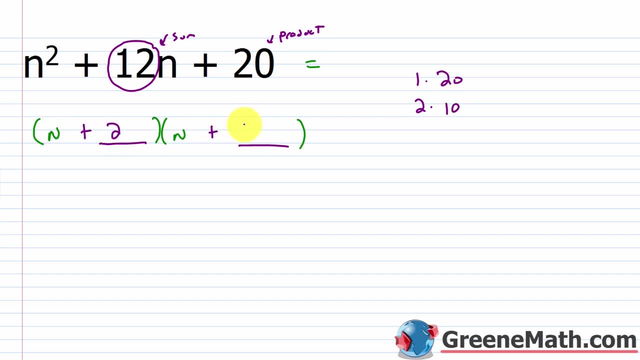 is 12.. So n plus 2, n plus 10, right, Those two quantities. the quantity n plus 2 times the quantity n plus 10 would give you n squared plus 12, n plus 20 back. So in some cases we're going. 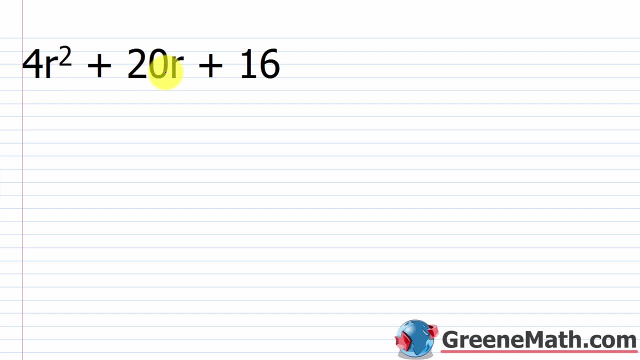 to have a common factor involved. So 4r squared plus 20r plus 16, there's a common factor of 4 that we can pull out And I'd be left with r squared plus 5r plus 4.. And this may trip you up, because if you're in this section, in your 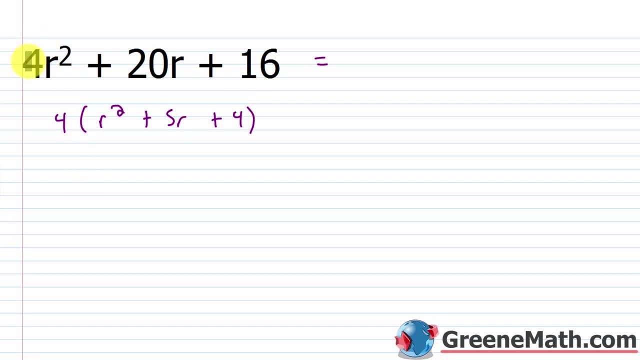 textbook and all of a sudden you see a coefficient that's not 1, you might say, well, I haven't gotten to that yet And that's a more difficult scenario. But a lot of times they're going to give you. 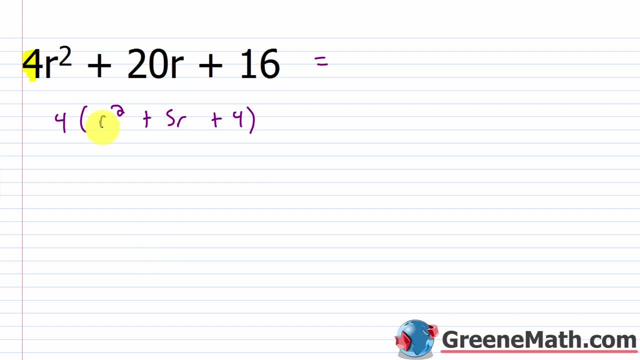 these problems to where you have to factor something out first and then you can use your normal procedure. So 4 just stays out there. You don't need to do anything with it. Just put the parentheses like you normally would, And then just think about what's inside here. OK, What's inside here. So I know if I have. 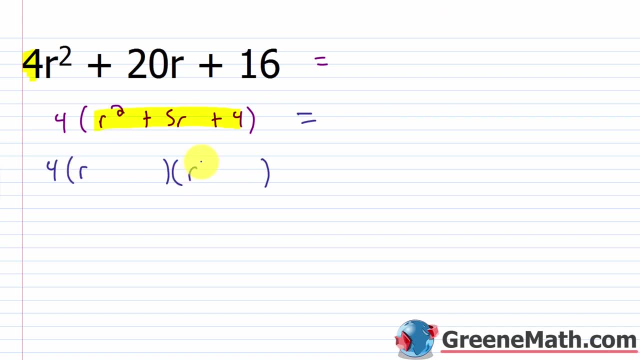 r squared, it's r and r. That's easy. Then I need two integers whose sum is 5.. So a sum of 5 and a product of 4, OK, A product of 4.. So that's really easy, because if you think, 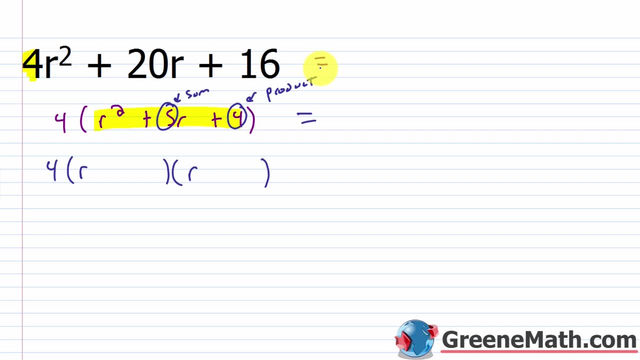 about 4, it's really 1 times 4 or 2 times 2.. 2 plus 2 is 4.. That doesn't work, So you don't have to think about the sum, So I'd have to go with 1 and 4.. If I do, 1 times 4,. 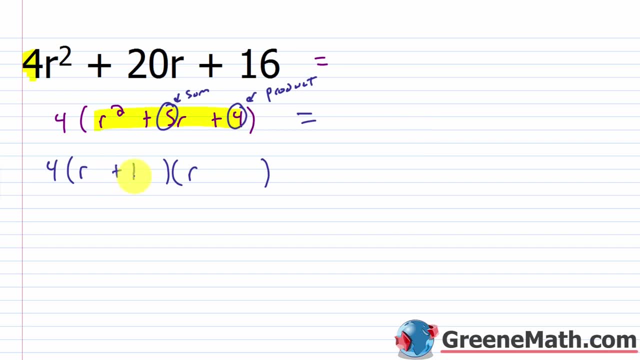 that's 4.. 1 plus 4 is 5.. So this would be plus 1, and this would be plus 4.. So I end up with 4 times the quantity r plus 1 times the quantity r plus 4.. 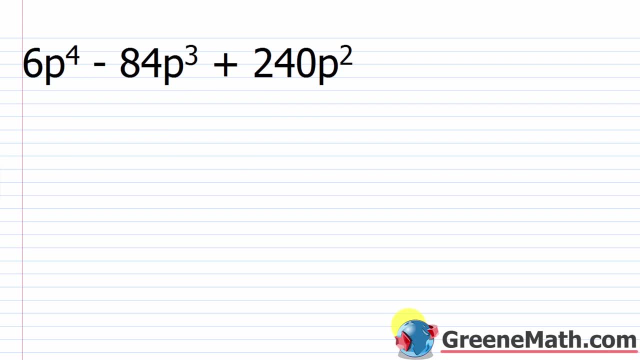 All right, let's take a look at another one like that. So we have 6p to the fourth power, minus 84p cubed, plus 240p squared. So obviously, if this is supposed to be a 1, here the coefficient. 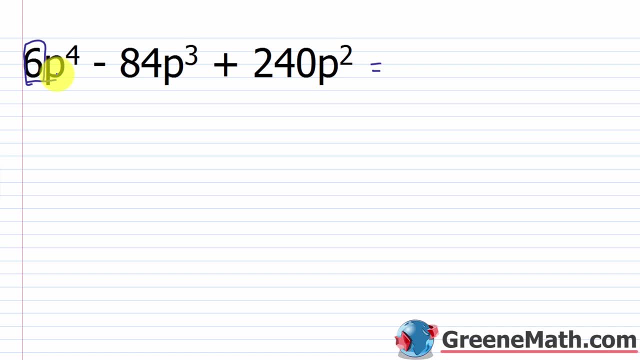 for the leading term it's going to be 2p squared, So obviously if this is supposed to be a 1 here, the coefficient for the leading term, we've got to do some additional work. So I noticed that I can pull out a 6p squared. 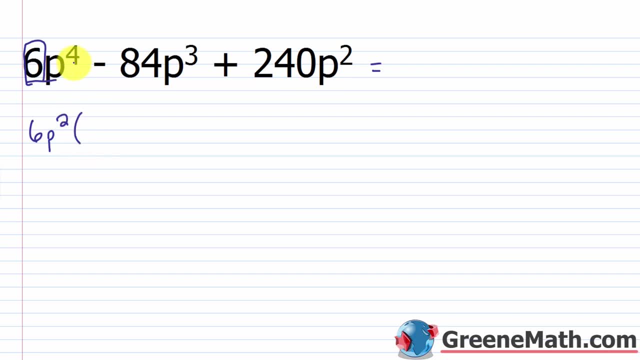 from everything. And so what would happen is this would be p squared, then minus This would be a 14p, then plus This would be 40, and then we could close our parentheses. Now, all I need to do is think about factoring this guy now, and let's just set this up. 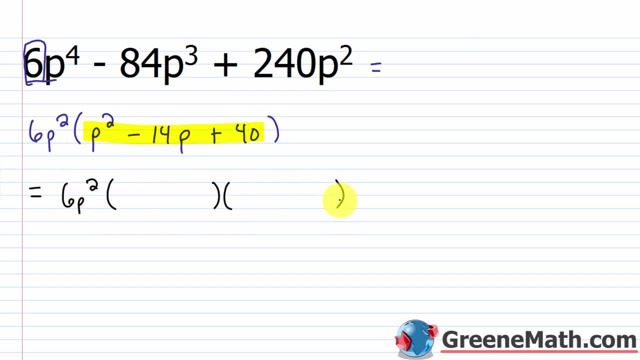 So we'd have 6p squared. then set up your parentheses Again. if I'm factoring this, and p squared is the leading term, this is p and this is p. For these positions here, I just want two integers whose sum is negative 14 and whose product is 40. Now that's really easy. 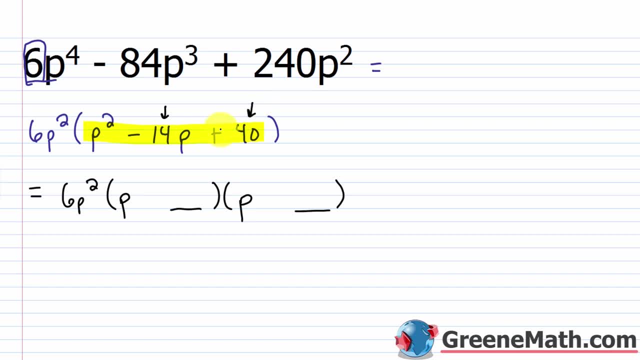 when you think- because I know that again, if I have a positive for my product and a negative for my sum, I know I need a negative and a negative- And just think about 40. You think about 4 times 10.. If I did negative 4 times negative, 10, that's positive 40. 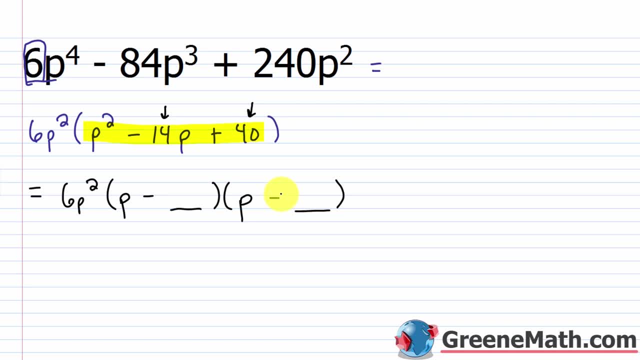 If I did negative 4 plus negative 10, that's going to give me negative 14.. So p minus 4, and then p minus 10 there. So 6p squared times the quantity p minus 4, times the quantity p minus 10.. 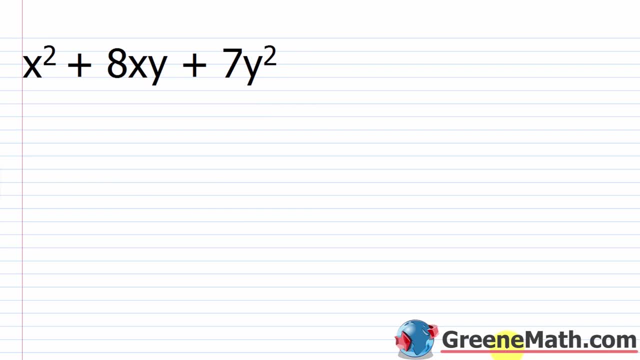 All right. so let's talk about another scenario that confuses people a lot. You might see two variables involved. So let's say you come across something like x squared plus 8xy plus 7y squared And you go: how in the world am I going to factor that? And it's actually. 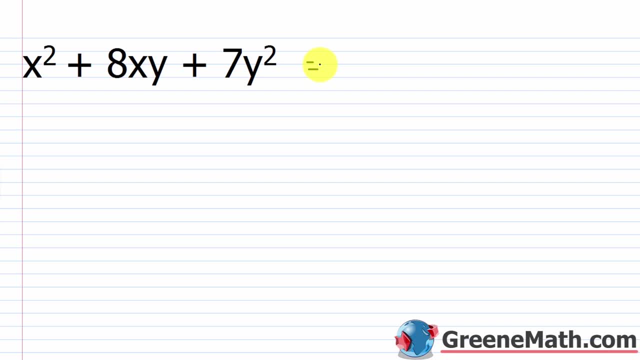 no more difficult than what you've just been factoring. If you just set up your parentheses and you just think for a minute, We know that the first term here times the first term here will give me x squared, And that's how I have x times x. Well, if I know that this is the 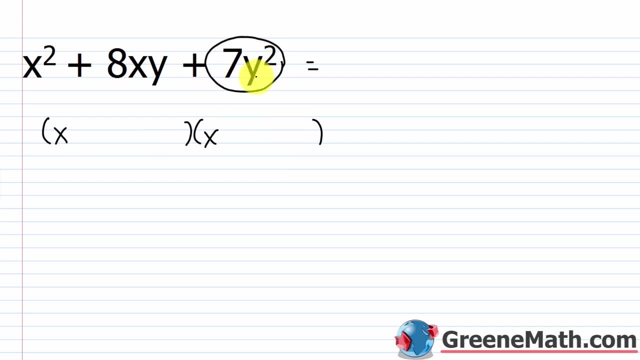 result of multiplying this times this. I know that that's going to come from y times y. Now, if this is set up, I just need to figure out what the coefficient of y is there and there, Because the outer and the inner will have xy and the inner will have y. So if I 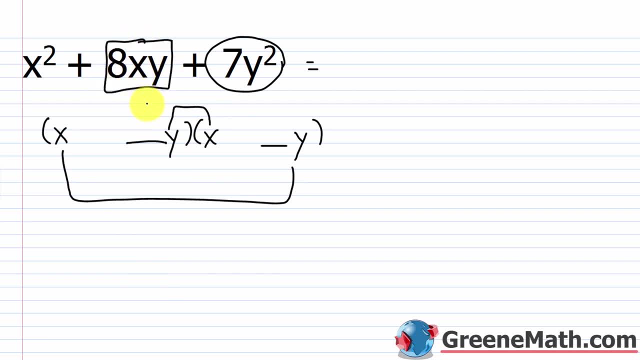 have y involved, so that's going to give me this right here. I just got to get the coefficient for y worked out in each case, And I do that the same way. Forget about that second variable. I don't even care about it, I've already set it up for myself. So all. 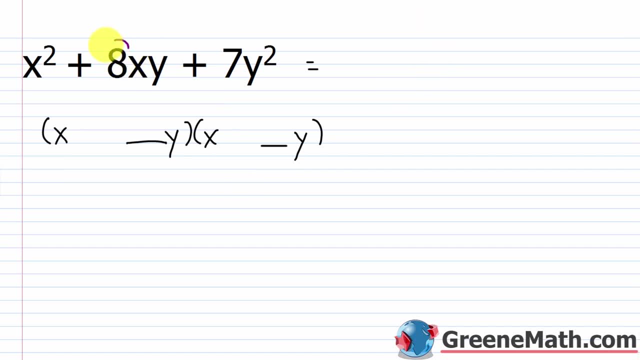 I need to really do is say: give me two integers whose sum is 8 and whose product is 7.. Well, that's easy. 7 is prime, so it can only be 1 and 7. And that works out. 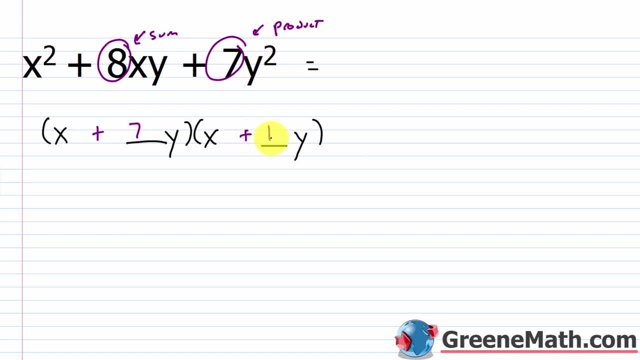 So put plus 7.. Put plus 1.. So you have the quantity x plus 7y times the quantity x plus 1y, or just x plus y. And check that through: FOIL x times x is x squared, Your outer will. 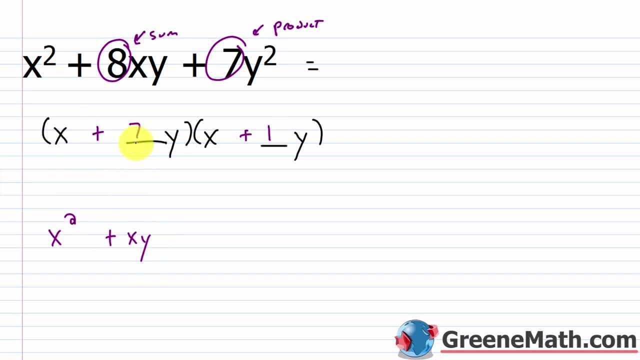 be x times y or plus xy, Your inner will be 7y times x or plus 7xy, And your last will be 7y times y, which will be plus 7y squared If you combine like terms here. so 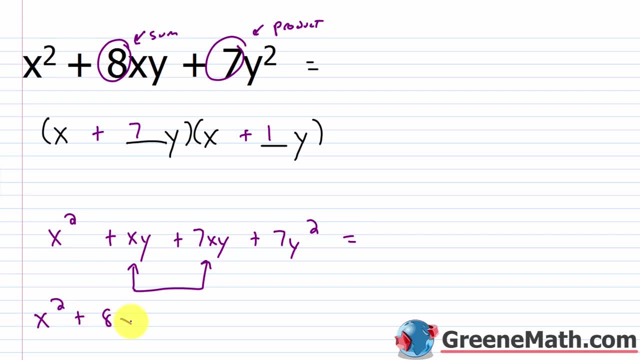 you'd end up with x squared plus 7y squared. So I can just figure out the proof of all this. Auf Wiedersehen, 8xy plus 7y squared, which is exactly what you started with right there. So if you have two, 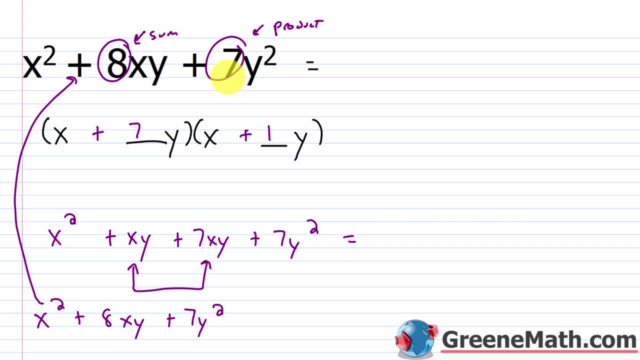 variables involved. don't panic, It's just as easy. Just make sure you figure this part out and this part out before you move on and figure out that sum and product part that we've been talking about for the whole lesson. Let's take a look at one last problem, And then we're going. 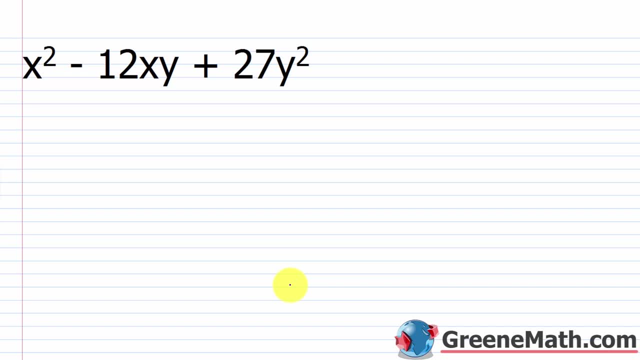 to talk about prime polynomials, And I'll just give you one example of that. So we have x squared minus 12xy plus 27y squared. So again, if I see two variables involved, I'm not going to panic. Set up your parentheses, I know that this would be x and this would be x. And if I have a y? 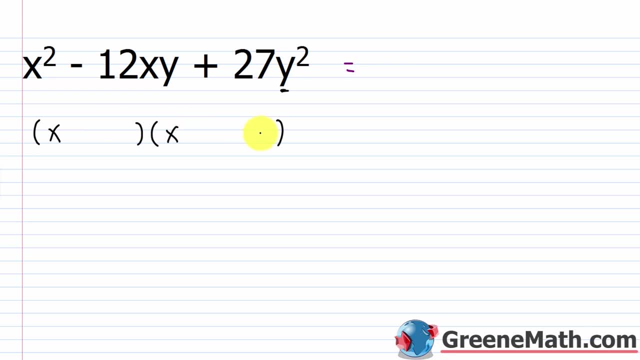 squared in the final position here. I know that came from this times this, So I'm just going to put a y here and a y here, And then I just say, okay, well, two integers whose sum is negative 12. This is my sum and whose product is 27.. So this is my. 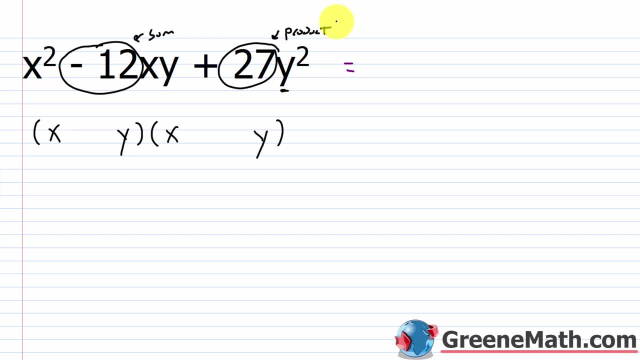 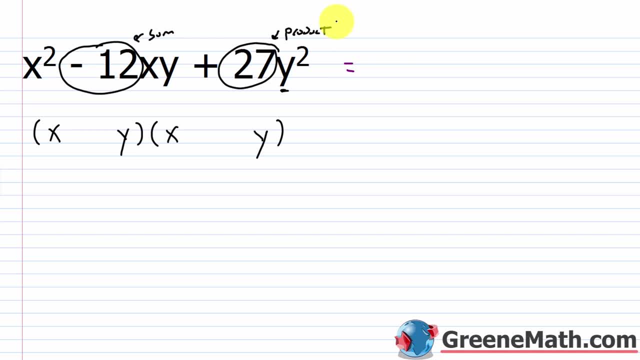 27. 27, I could do 1 times 27,, or I can do 3 times 9.. Now I've got to work out some things with the signs here, because I've got a positive product and a negative sum, So that means I want a negative. 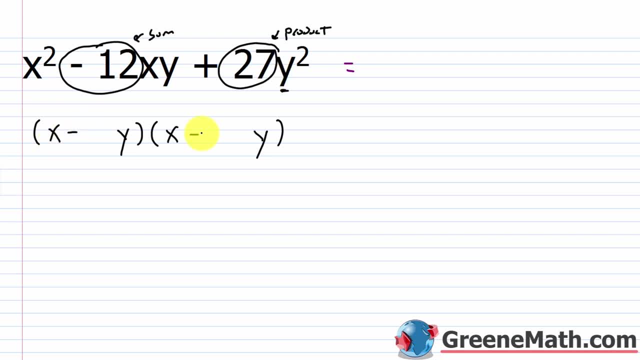 and another negative. Negative times negative is positive, Negative plus negative is negative. So what I can do here is say a negative 3 and a negative 9. Negative 3 times negative, 9 is positive 27.. Negative 3 plus negative 9 is negative 12. So I would have the quantity x minus 3y. 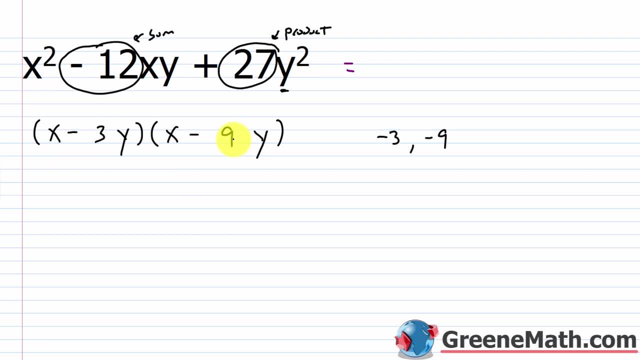 times the quantity x minus 9y. Okay, super, super simple. Now let me give you an example, real quick, of something that's prime. You're going to come across these polynomials that you just can't factor. Okay, so let's say I have something like x squared plus 7x plus 14.. And I said: 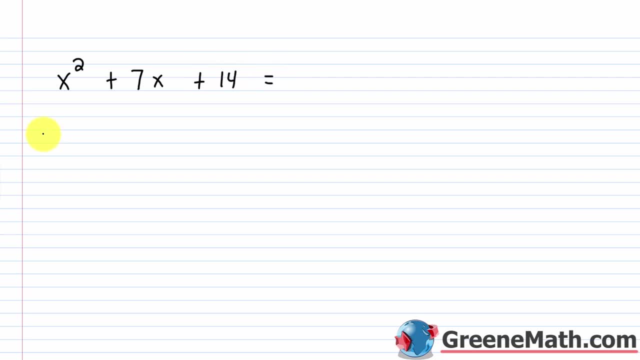 go ahead and factor that for me. Well, you go ahead and start out by saying: okay, well, I can do that. x and x, that's going to be leading. And then two integers: who's what? Whose sum is 7, whose product is 14.. So this is the sum. 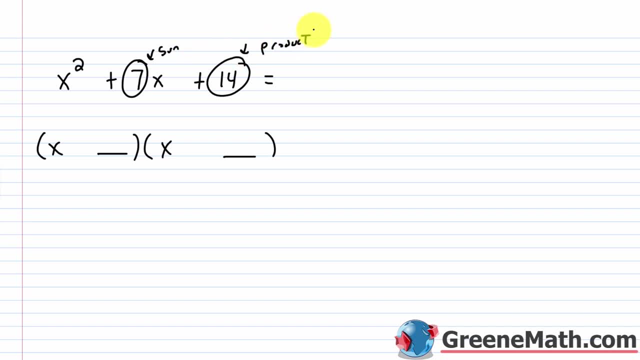 and this is the product. This is a great example to do this, because it's very easy, Because 14 really is what It's only 1 times 14, or 2 times 7.. Now, if I add 1 and 14, I get 15.. 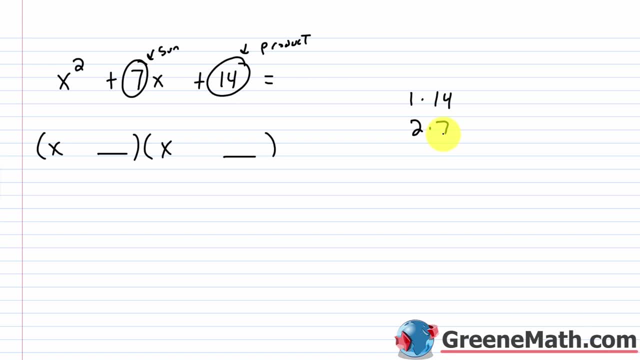 That doesn't work. If I add 2 and 7, I get 9.. So that doesn't work. So there's no configuration that would work. And because this is positive and this is positive, I know the signs for the integers have to be positive, So really I'm out of options. 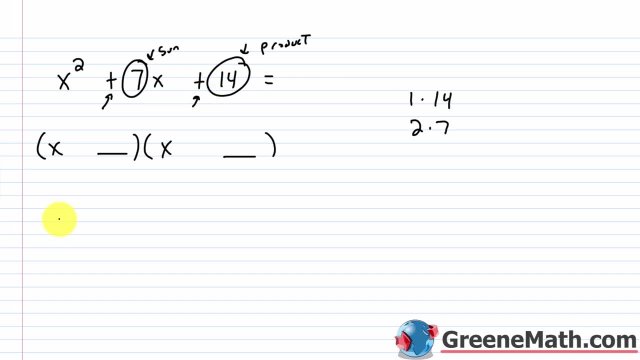 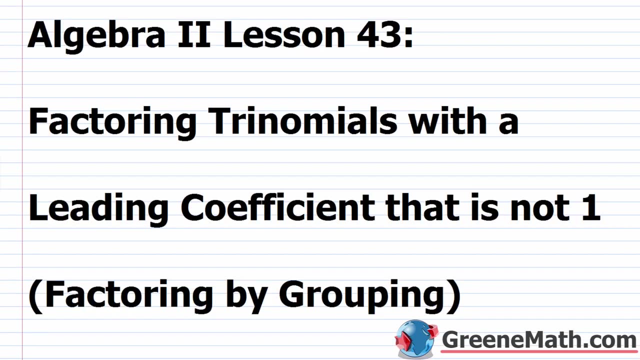 here And I've got to stop and say: well, this polynomial is prime, This is prime And using rational numbers, I will not be able to factor this. Hello and welcome to Algebra 2, Lesson 43. In this video, we're going to learn about factoring trinomials with a leading coefficient. 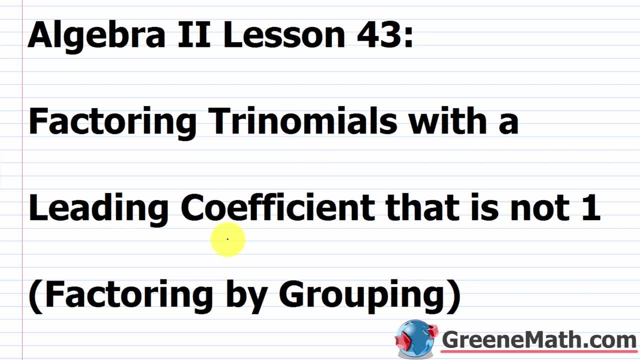 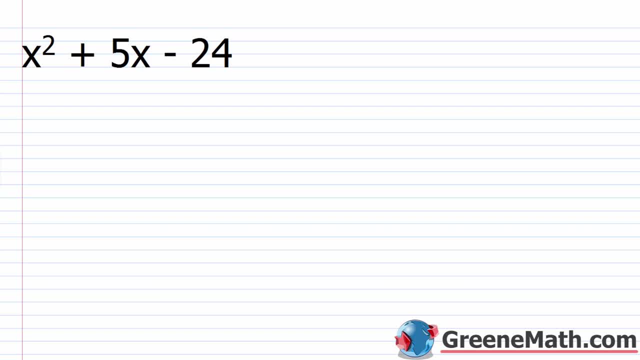 That is not 1.. And we're going to be using the factoring by grouping method. So in the last lesson we reviewed how to factor a trinomial with a leading coefficient that is 1.. So this is by far the easiest scenario you're going to come across. So I have an example of that. So let's say you: 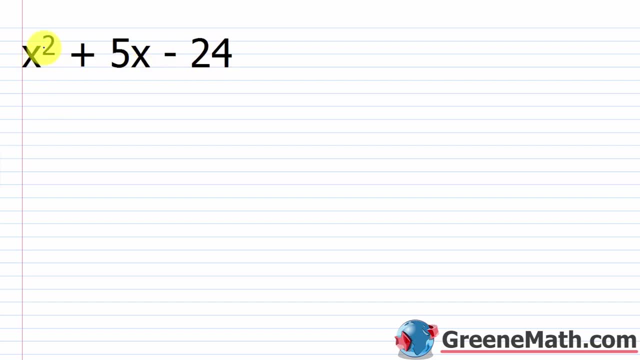 had something like x squared plus 5x minus 24.. And here you can see the leading coefficient, or the coefficient for the squared variable. x is a 1.. If nothing's displayed there, the coefficient is 1.. And so we're going to use the factoring by grouping method. 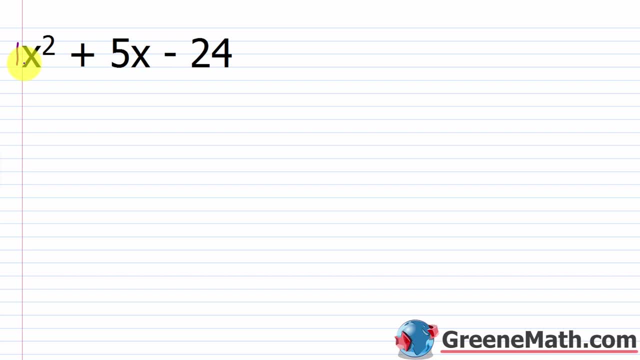 So in this particular scenario, it's very easy to factor this into the product of two binomials. I can just set up my parentheses And I don't know if I have x squared. The first position here is x, and the first position here is x as well. x times x would give me x squared. Now, the only thing that 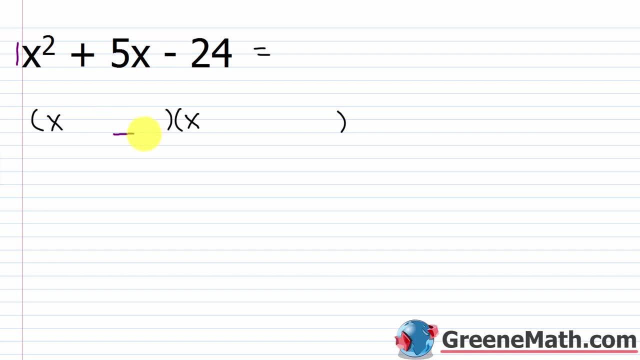 I really need to figure out is what goes here and here, And to do that, I think about two integers whose sum is 5. And I'm going to use the factoring method to figure out what goes here and here. So I can just write that one of these is positive and one of these is negative, And I can just think. 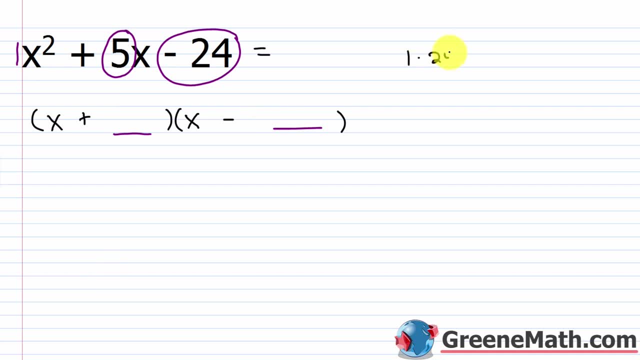 about factors of 24.. I've got 1 times 24.. I've got 2 times 12.. I've got 3 times 8.. Now when I see something that I know in my mind, those two integers, if I put them together they're going to be. 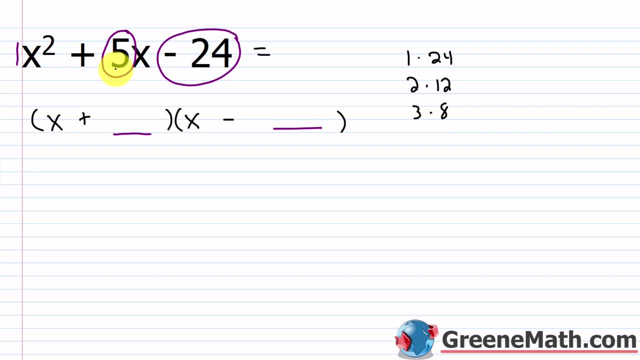 positive. So I can just write that one of these And I can just set up my parentheses And I can around the signs could get me to 5.. I just stop right. 3 and 8, if I play with the signs will. 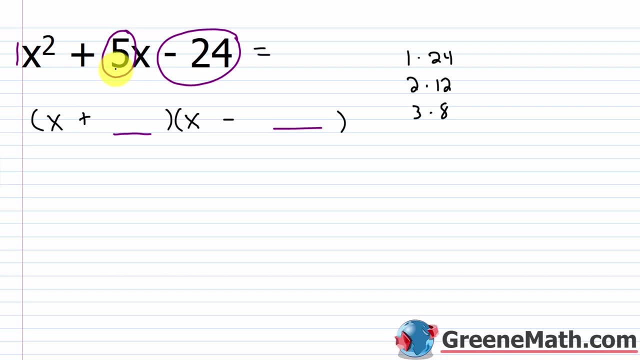 work If I had a negative 3 and a positive 8,. well, negative 3 times positive 8 would give me negative 24.. Negative 3 plus 8 would give me positive 5.. So I know I want x plus 8, and I want 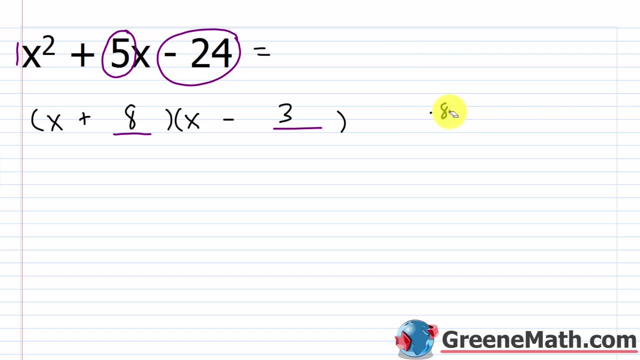 x minus 3.. So that's how you go about factoring these easy scenarios. Not a whole lot of work. You just have to go through the factors And figure out what two integers again sum to this the coefficient for the variable, that's. 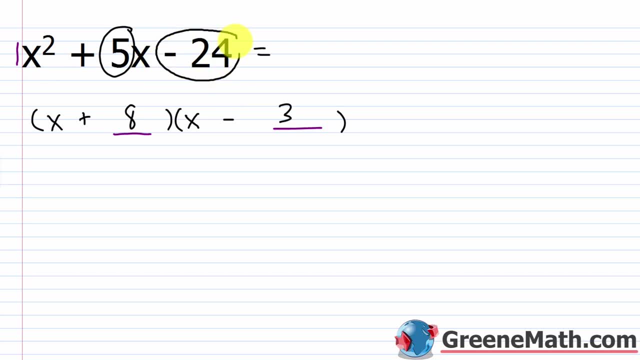 raised to the first power and have a product of this, your constant at the end. Now, what we're going to look at today is something that's a little bit more challenging. What if we have a scenario where the coefficient on the squared variable is not a 1?? So in this example, I have 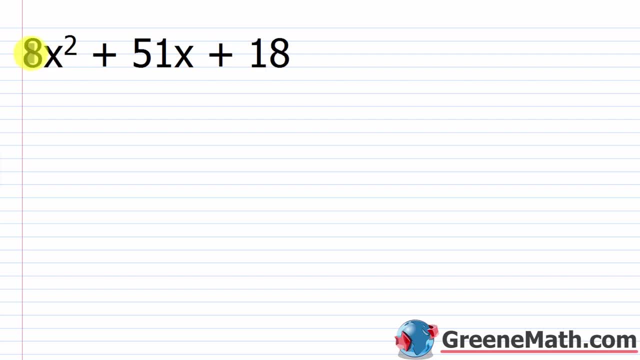 8x squared plus 51.. X plus 18.. So you notice that this is an 8 here. So I can't just go ahead and set this up and say, OK, well, I have x times x. That's no longer going to be the case, So now, instead of just having to, 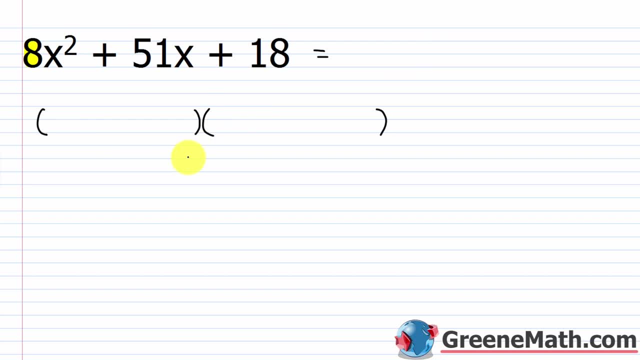 find 2, I have to find all four positions. So how can we do this? Well, there's two main methods that are taught in every textbook. One is going to be reversing the FOIL process, which I personally don't like. 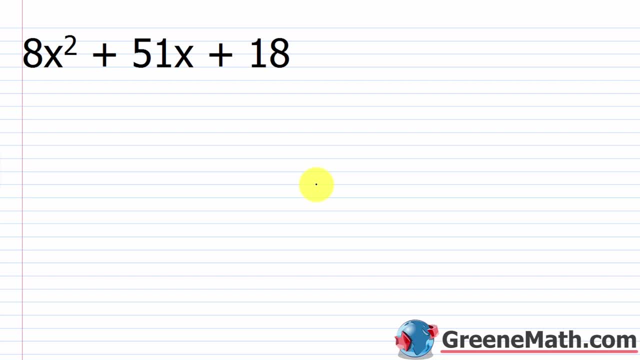 And the other is going to be a method that relies on factoring by grouping. Now, I like this method. I think it's quicker and more efficient, So I'm going to start by teaching you that in this lesson, And the next lesson I'm going to cover reverse FOIL. All right, So the first thing you need to 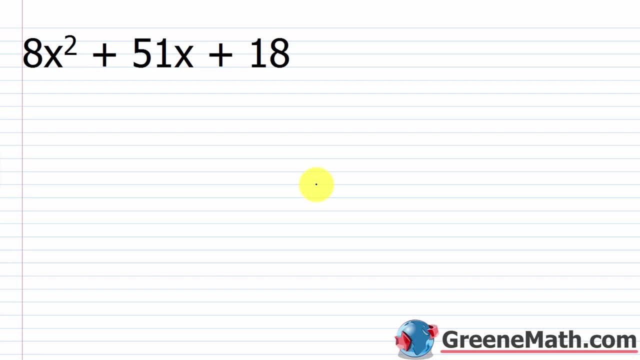 understand is that in your textbook, when they're teaching this method, they're always referring to A, B and C, And you need to know what those are. So generically, when we see a trinomial, we generally see ax squared plus bx plus c. So what does A represent? A represents this. 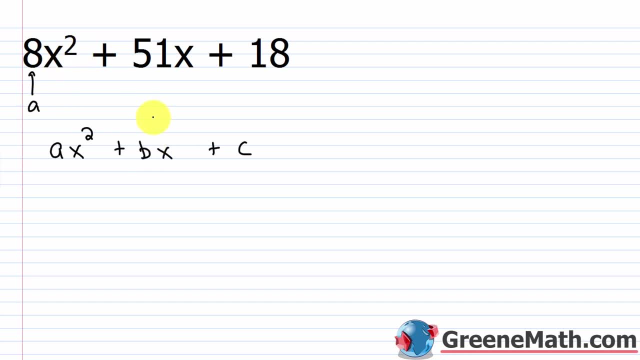 It's the coefficient for the squared variable. Then what does B represent? B represents this. It's the coefficient for the variable raised to the first power. And then what does C represent? C represents this. This is the constant. So if your book says something like we want to find two, 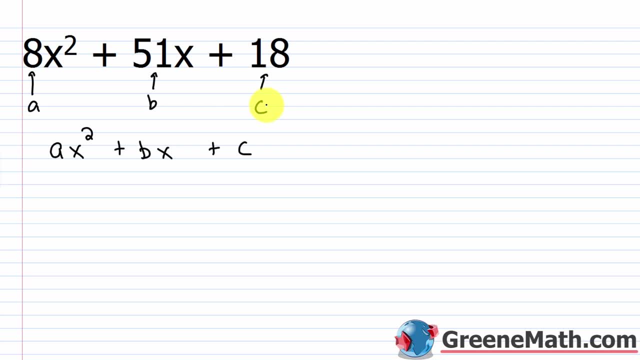 integers whose product is ac and whose sum is b. Well, I know that a product of ac is what. Well, A is 8 in this case, And C, in this case, is 18.. So I would need to multiply 8 times 18. And that would give me 144.. And then a sum of b. 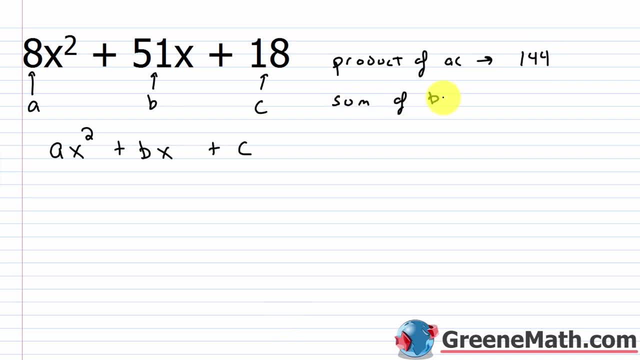 a sum of b. Well, b is 51.. So what I'm going to do here is I'm going to think about some factors, and I could do that with a factor tree, or I can kind of do that by just going through things. 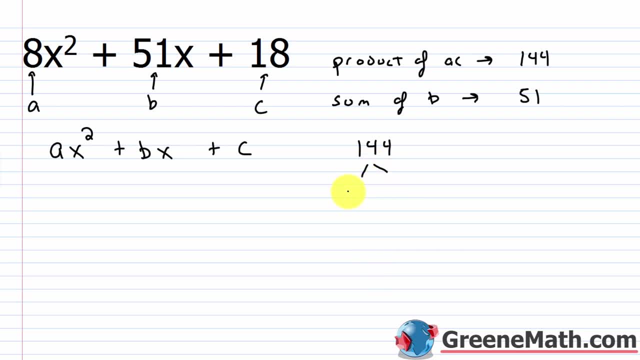 It doesn't really matter. Let's just make a factor tree: 144 is what 12 times 12.. Most of us know that. And then 12 is what It's 4 times 3. We know 3 is prime And then 4 is 2 times 2.. 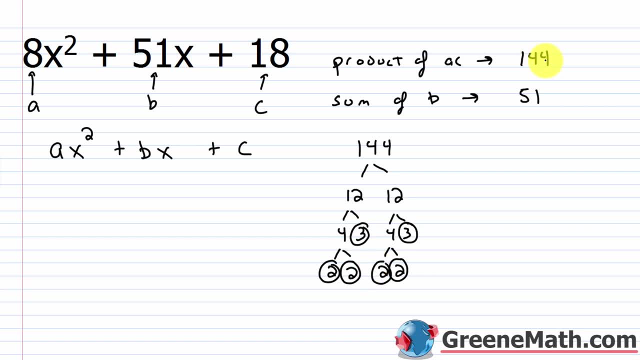 So, to go through this, I can think about two integers whose product would be 144 and whose sum would be 51.. OK, Well, we could start with 1 times 144.. That's obviously not going to work. You can just mark that out. 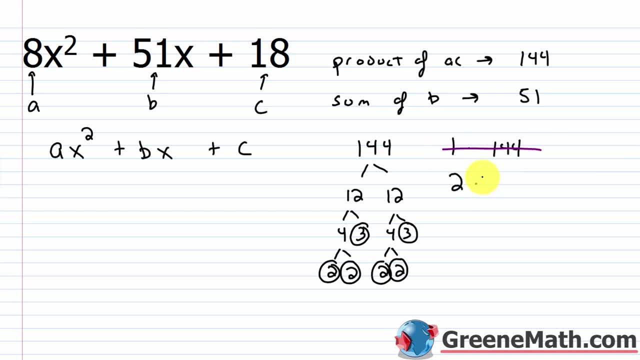 Then you could go on to, let's say, 2 times 72.. Again, that's not going to work. Mark that out. Then is it divisible by 3?? Yeah, of course it is. So I could do 3 times 48.. 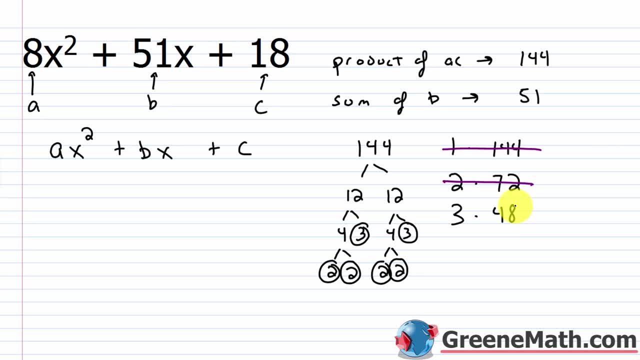 Now let me stop for a second. When you see something like this and you say, okay, well, 3 and 48,. if I had 3 plus 48, that would in fact give me 51. So it's just a matter of going through the factors. 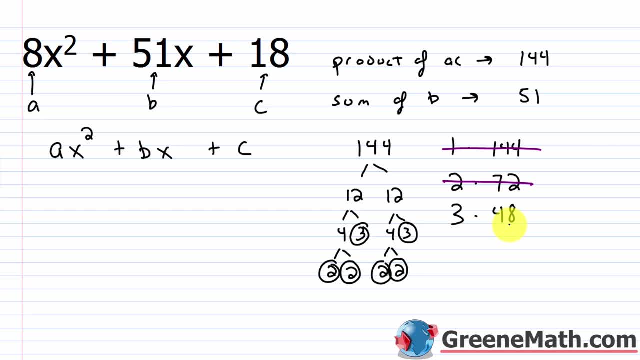 until you get the two integers that you need. So once I know that I need 3 and 48, it's a little bit of a different process from before. Let me kind of erase this. I'm going to say my two integers are positive 3 and positive 48. 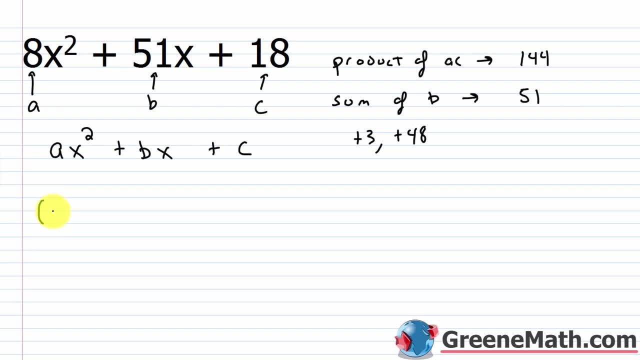 So for some of you, you'll stop and you'll say, okay, well, I figured it out. This is going to be x plus 3,, that quantity times the quantity x x plus 48, and I'm done. 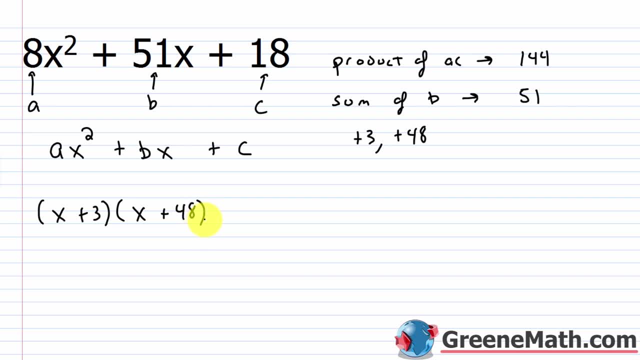 Well, no, not exactly. Okay, You need to take this information right here and use it to rewrite this polynomial here. Okay, Remember, when we use factoring by grouping- and I'm just going to erase this real quick- when we use factoring by grouping, 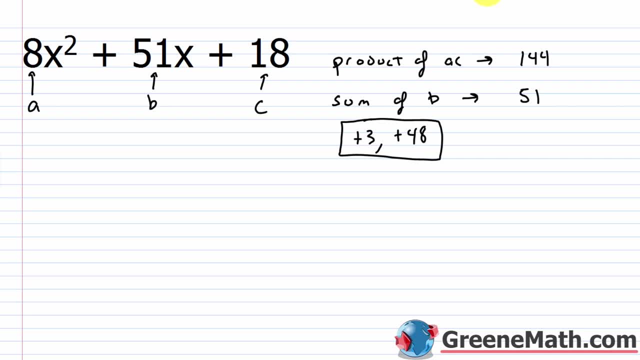 we are generally factoring a four-term polynomial. So what I want to do is I just want to make this trinomial into a four-term polynomial, And the way I'm going to do that is I'm going to rewrite this middle term. 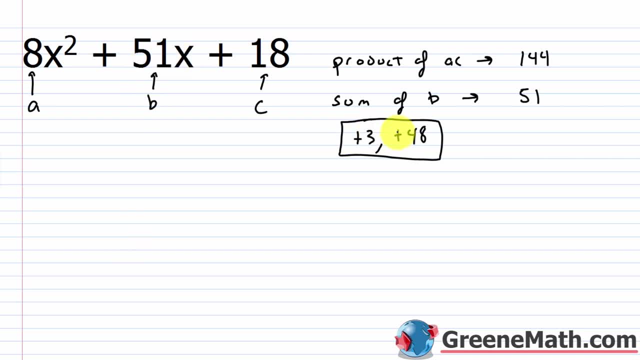 this 51x using these two integers. So I would have 8x squared. I'm going to put plus 48x, Then I'm going to put plus 3x and then plus 18.. So, mathematically, have I done anything illegal? 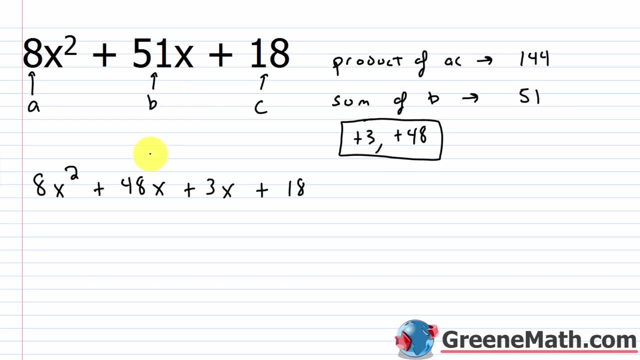 No, because 51x is the same as 48x plus 3x. So I've just rewritten this. I've just rewritten this polynomial as a polynomial with four terms. Now, once I've done that, what you're going to see is: 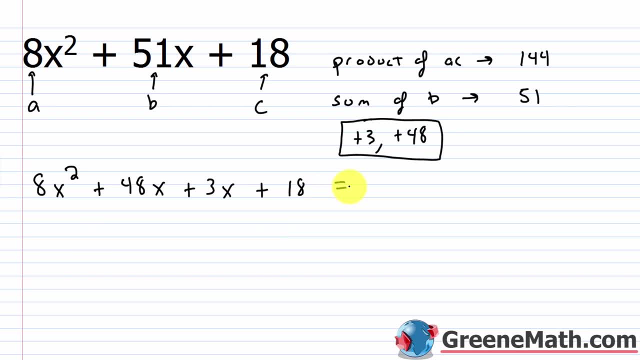 that you can use factoring by grouping now to get this into the product of two binomials. So from the first group I could pull out an 8x. What would be left is what You'd have: x plus 6.. 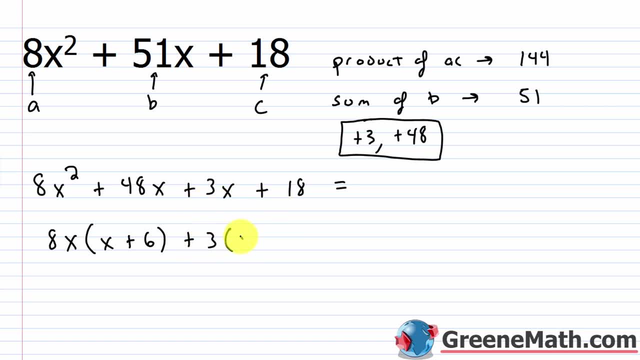 From the second group, I could pull out a 3. What would be left is x plus 6. So I have a common binomial factor. I have a common binomial factor of x plus 6.. So if I factored that out, what would I have? 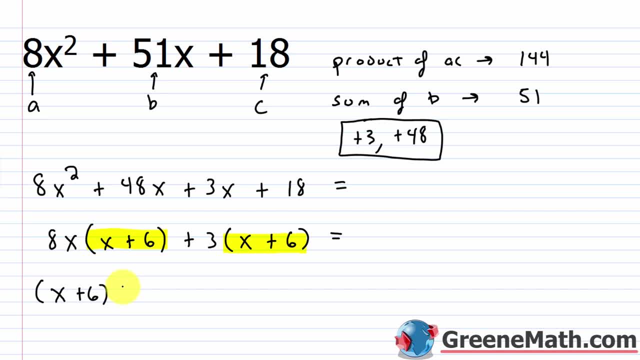 Well, I'd have x plus 6, that quantity times what's left. You'd have 8x plus 3.. So the quantity x plus 6 times the quantity 8x plus 3.. Now I'll leave it up to you to pause the video. 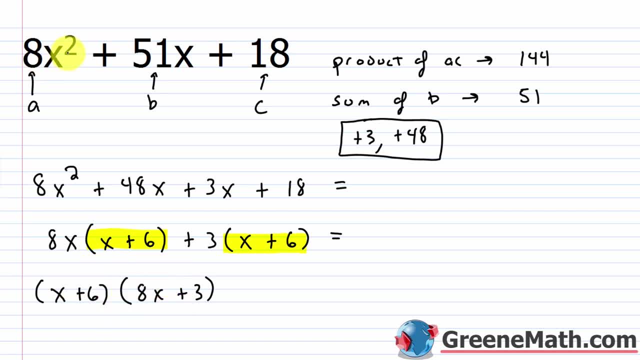 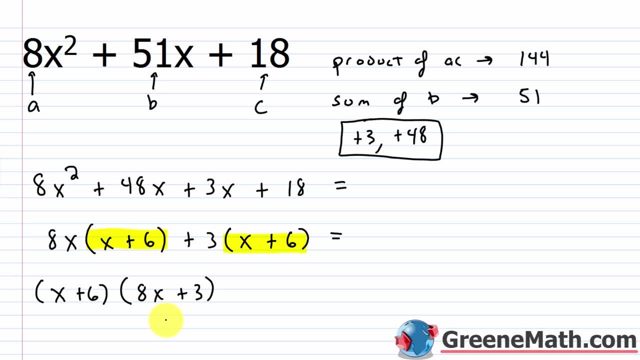 I'm going to go ahead and do that. Integers are that you're trying to find, but it is something that you can go step by step on. All right, let's take a look at another one. So we have 10x squared plus 43x minus 9.. 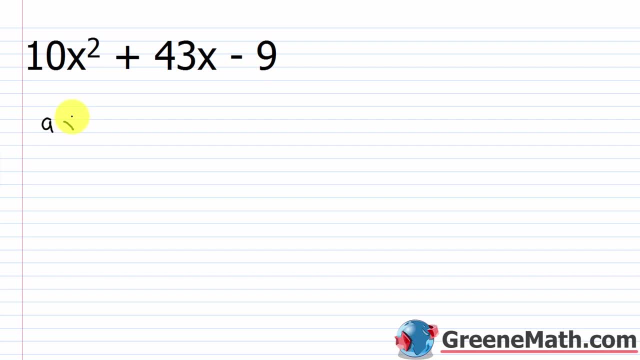 Again, just for the first few. I want to just identify things. So this is ax squared plus bx plus c, So a here is 10, b here is 43, and c here is negative 9.. Okay, the negative and the 9.. 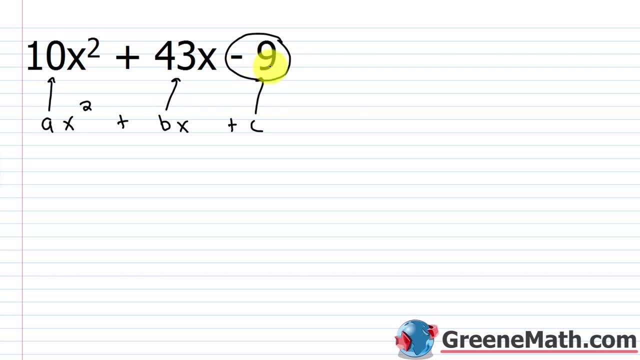 That's why I circled it. So if I want two integers, whose product? again the product is AC. So what is A? It's 10.. What is C? It's negative 9.. So AC would be 10 times negative 9.. That's going to be negative 90. And we want a sum of 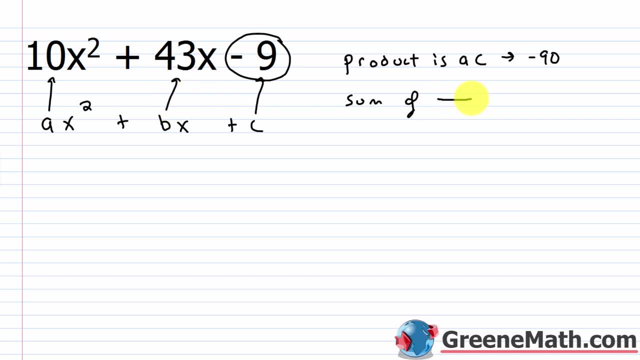 this middle term B, So a sum of 43.. All right, In order to figure this out, I think about the factors of 90.. Forget about the fact that it's negative 90. Just think about 90 for a second. 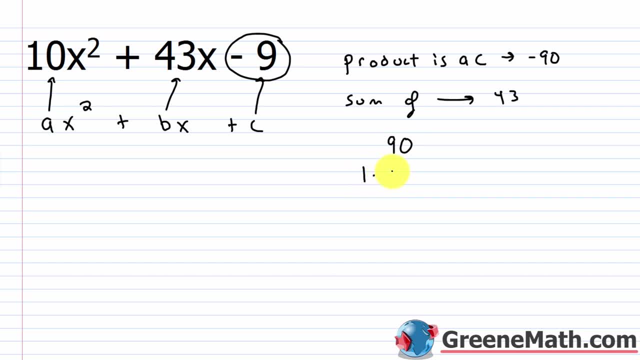 90 is pretty easy. I don't need to really make a factor tree. You've got 1 times 90. And again you've got to flip the signs around and make this work because this is going to be a negative product. But I already know that this won't work out because it's never going to sum the 43. no. 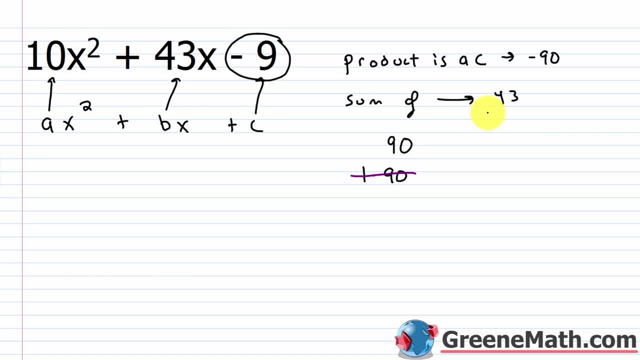 matter how much I change the signs around, Then the next thing I would say is 2 and 45. So 2 times 45. Well, immediately, I've found something that would work. If I did a negative 2 and a positive 45,. well, yeah, 45 minus 2 is 43.. That's what I'm looking. 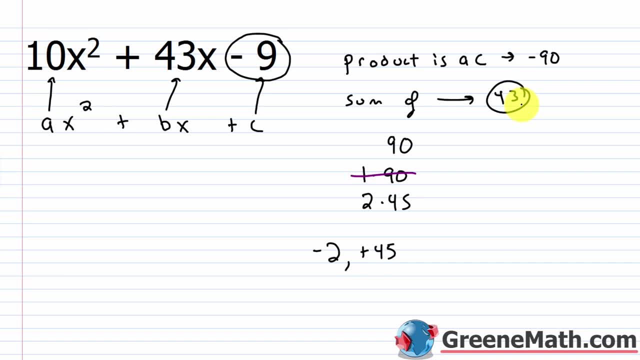 for, And then negative 2 times positive. 45 is negative 90.. That's what I'm looking for there. So remember I'm not done. once I've figured this out, I've got to use this information to rewrite this middle term. So what I'm going to do is I'm going to say I have 10x squared. 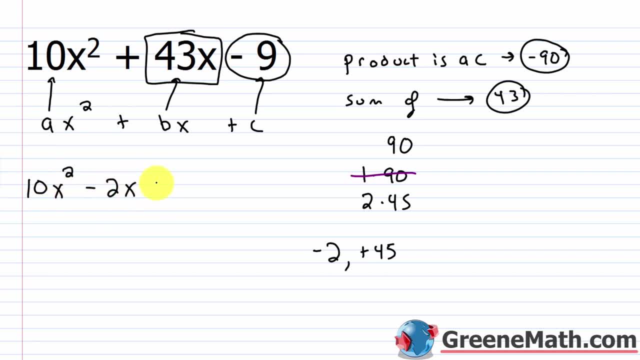 I'm going to do minus 2x, Then plus 45x and then minus 9.. All right, So once I've rewritten this trinomial as a polynomial with four terms, again I can use factoring by grouping. So let me erase this. 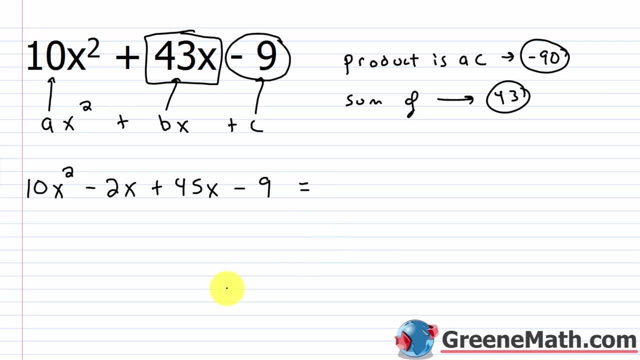 and we'll set this up. So from the first group I could pull out a 2x. So pull out a 2x, I'd be left with 5x minus 1.. From the second group, I could pull out a 9.. 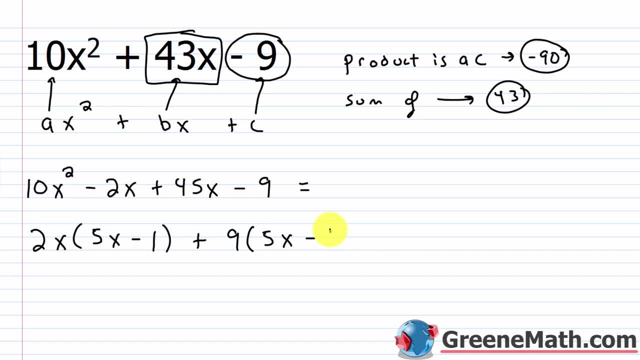 I'd be left with 5x minus 1.. So you see, I have a common binomial factor of 5x minus 1.. And we can just factor that out. So we'd have 5x minus 1, that quantity times the quantity 2x. 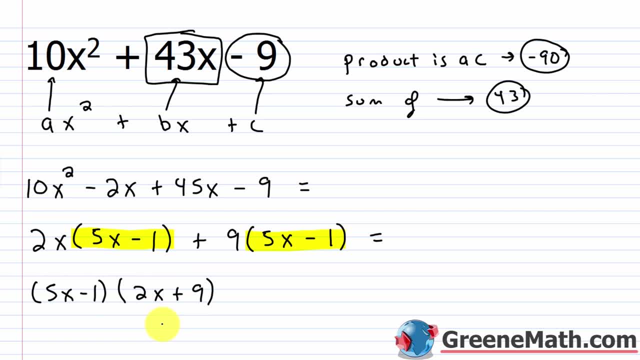 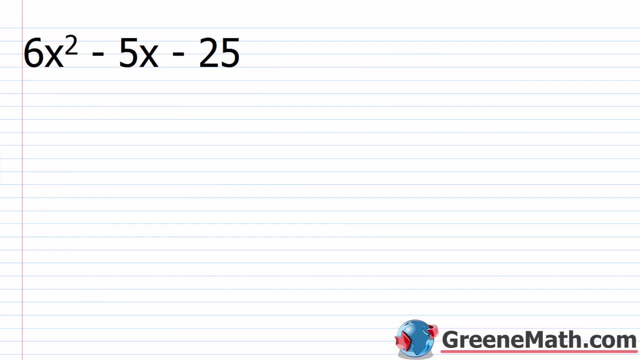 plus 9.. So this is our answer: the quantity 5x minus 1 times the quantity 2x plus 9.. All right, Let's take a look at another one. So we have 6x squared minus 5x minus 25.. 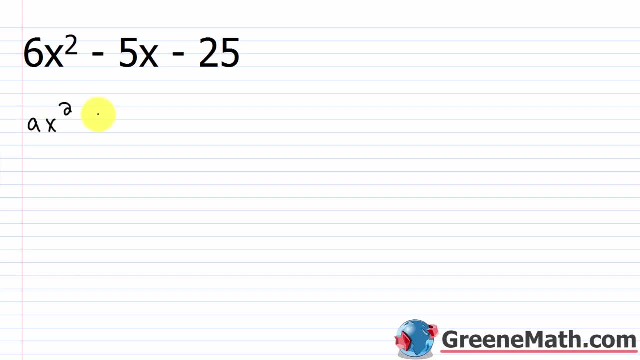 So again, let me just label things. So this is ax squared plus bx plus c, This is a, this is b, In this case the negative and the 5. So I'm going to circle it, So that's clear. And this is c. 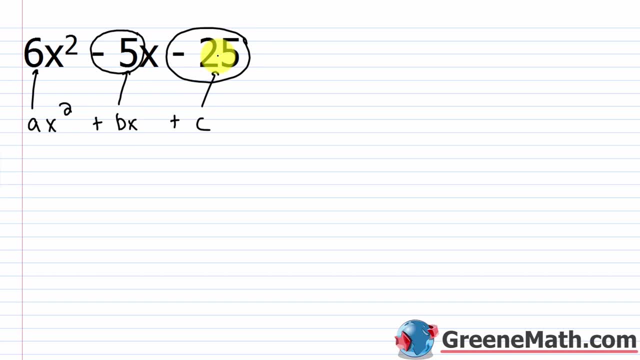 negative 25, the negative and the 25.. So again, if I want two integers whose product is ac, a is 6,, c is negative 25.. So 6 times negative 25 is going to give me negative 100.. 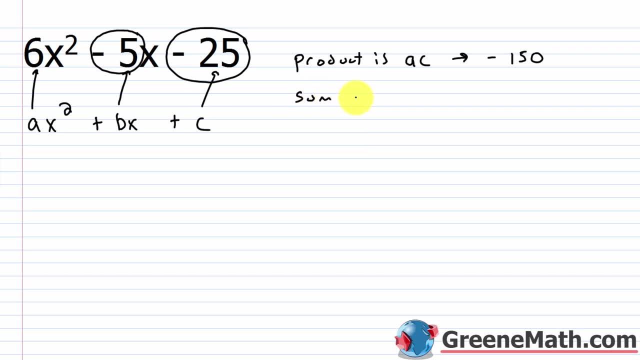 And then we want a sum, a sum of negative 5. So we think about factors of 150.. Forget about the negative for a second. Just think about factors of 150.. 150.. So you've got 1 times 150. Again, no way you can make the signs work there. Then you'd have 2 times 75.. 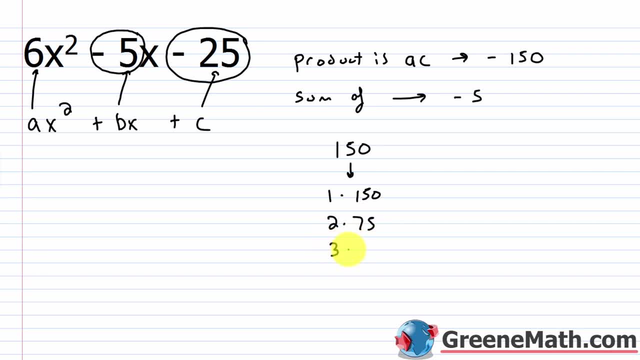 Can't make the signs work there. You would have 3 times 50. That's not going to work. You would have 5 times 30. That's not going to work. You would have 6 times 25.. Again. 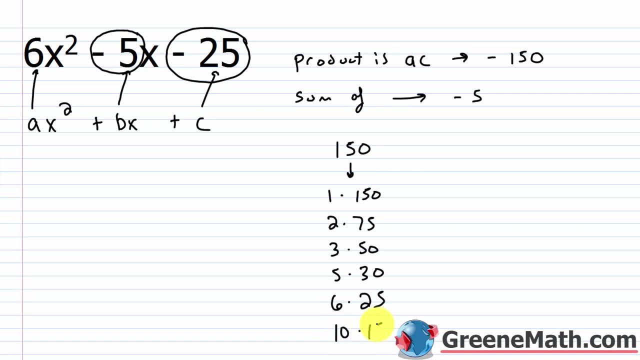 not going to work, Then the next one you come to would be 10 times 15.. If you think about this, I can make that work with the signs. If I had a positive 10 and a negative 15, I can make that work. So I'm always mentally kind of saying, okay, well, I know it would work. 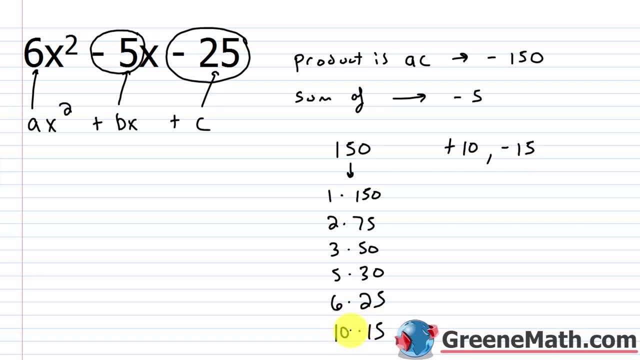 with the product. But can I mess with the signs here and make it work? Well, yeah, If I think about 15 minus 10 in my head, I get positive 5.. I know I need a negative 5, but I can just play with. 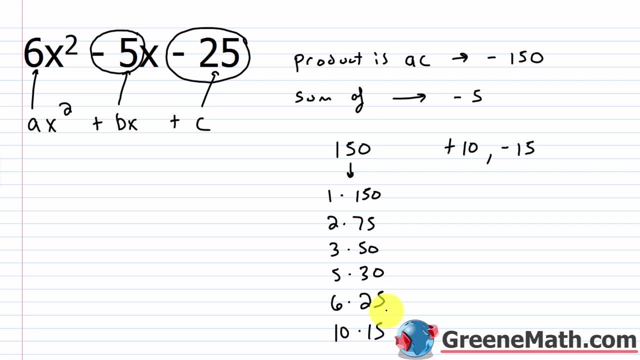 the signs and make that work. So that's kind of what I'm doing here. That's what I'm thinking about. So let me erase this. We found our two integers And again, I just want to rewrite this middle term. I want to rewrite negative 5x using these two integers. So I would have 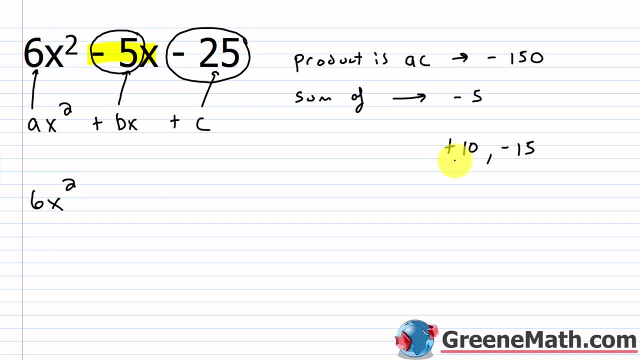 6x squared. I can say plus 10x. So I could say minus 15x Wouldn't matter. So let's just say plus 10x And then let's say minus 15x And then minus 25.. So, now that I've rewritten this as a four-term, 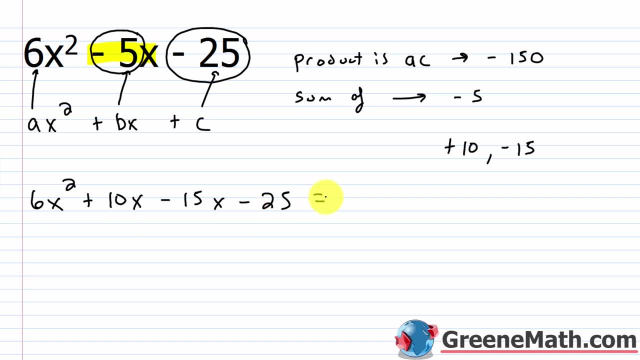 polynomial. I can use factoring by grouping. So from the first group I could pull out a 2x And I'd be left with 3x plus 5.. From the second group I would pull out a negative 5.. 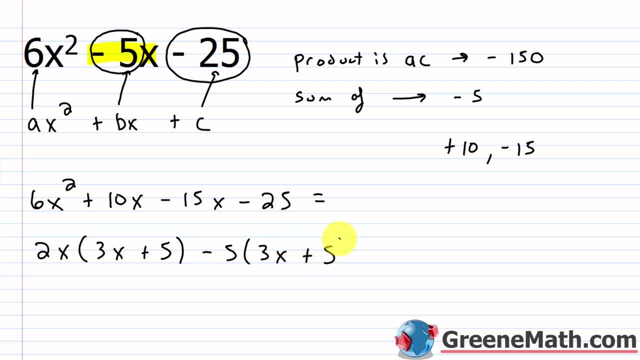 And I'd be left with a negative 5. And I'd be left with a negative 5. And I'd be left with a 3x plus 5.. So I have a common binomial factor of 3x plus 5. And of course I can factor that out. 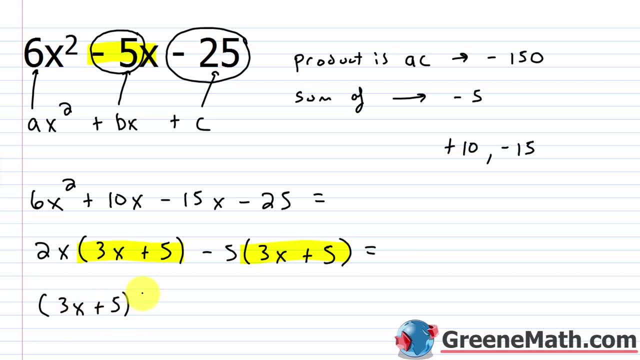 So I'd have 3x plus 5 here, that quantity, And then times what's left, we'd have the quantity 2x minus 5.. So your answer for this one would be the quantity 3x plus 5 times the quantity 2x. 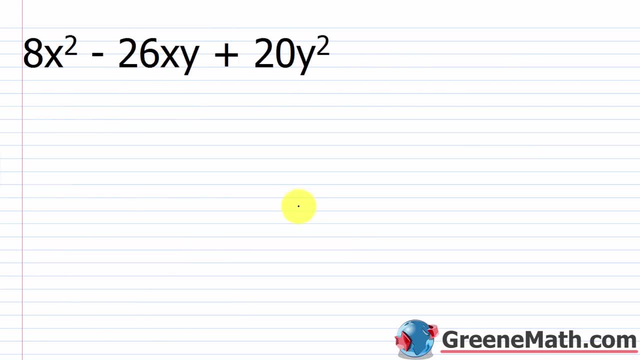 minus 5.. All right, for the next problem. I'm going to do something that's a little bit more challenging. A lot of students see these And they just shut down, And really you shouldn't, because the procedure is the same. It's no more. 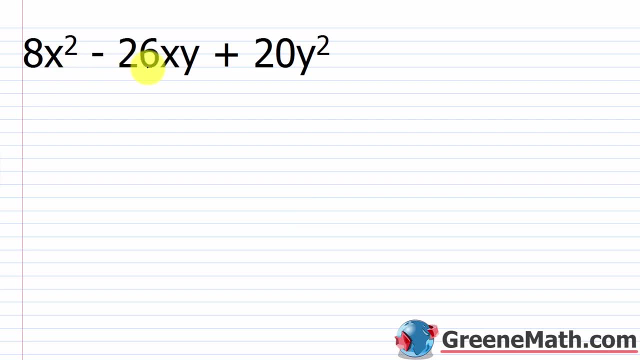 difficult. So let's say: you see something like 8x squared minus 26xy plus 20y squared. The first thing is that, notice, we have an even number here, here and here. So before I even start, I can pull. 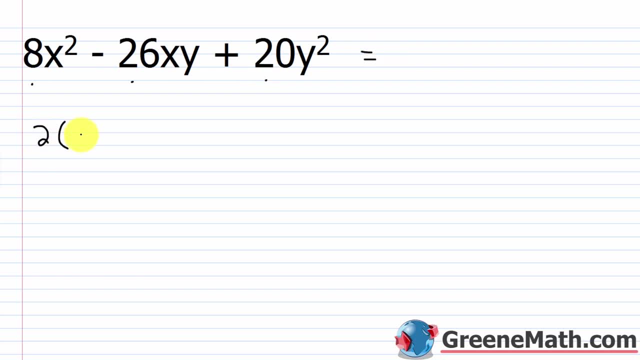 that out. So just pull out a 2.. So pull out a 2, you'd get 4x squared, then minus 13xy and then 4y squared. Now, once that's done, you think about the middle part here And again a lot of. 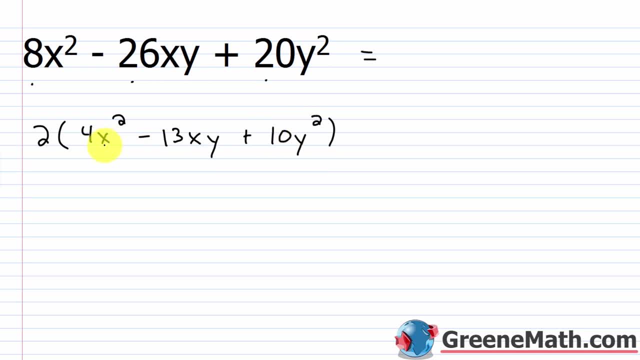 students freak out because they only have an x normally, or whatever the variable is. Now you have an x and you have a y to deal with And they're like: what am I going to do? There's two variables. I'm going to tell you what you can do. Don't even think about the second variable, Just. 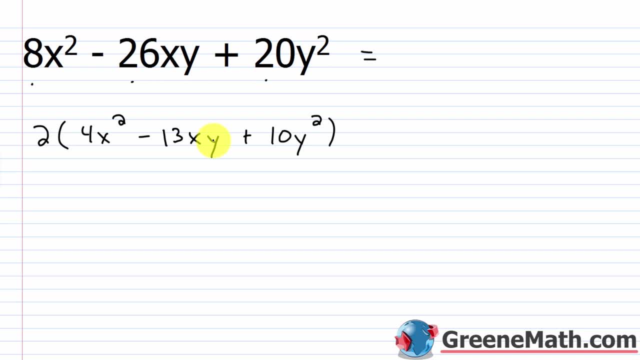 do your normal process And I'll show you how to work that variable in in a second. So if I just ignore the fact that I have a y, just kind of line it out for a second And just say: okay, well, if I had this scenario- 4x squared minus 13x plus 10, what would I do? I 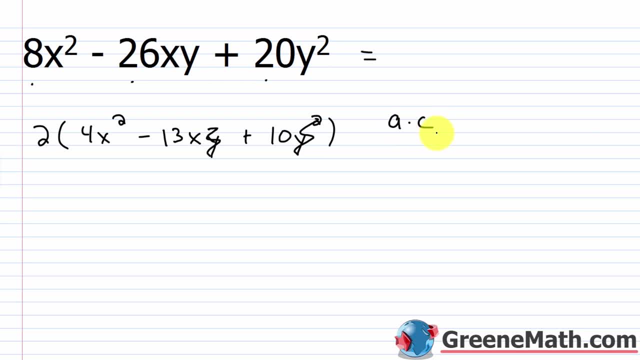 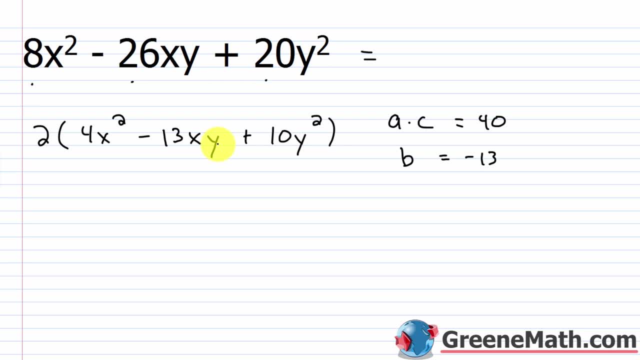 Well, b is now negative 13 times y. It's the coefficient for the x to the first power. So what's multiplying x to the first power? Well, negative 13 is, and also y is. So I can just say this is negative 13y. And then what's my term at the end here? Well, it's 10y squared, So normally. 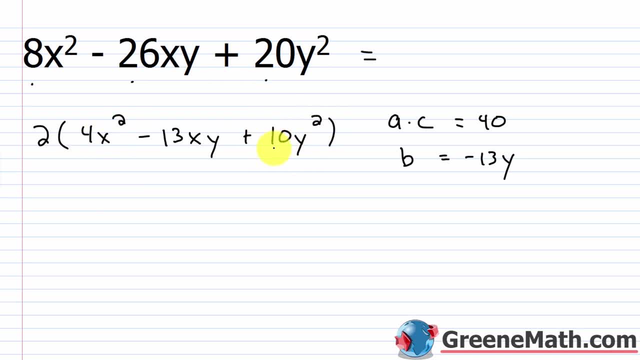 I do the coefficient for the squared variable times the term at the end. We can do that again. So 4 times 10y squared would be 40y squared. No more difficult. okay, You just include the second variable. Well, you could also just leave it off if you wanted to. 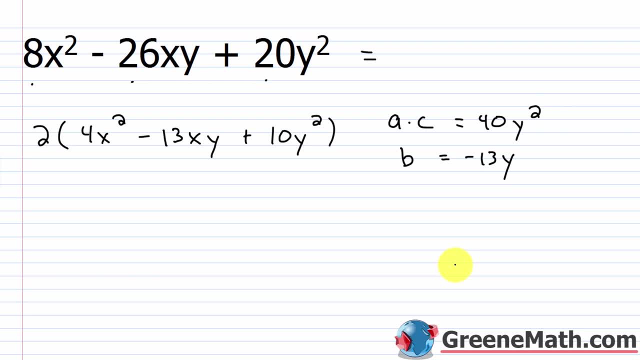 and just make sure that you put a y next to the two integers that you come up with, okay. So let me just say this: Find two integers whose sum is negative 13 and whose product is 40, and attach a y at the end of those two integers And I'll show you that that works. So for 40,. 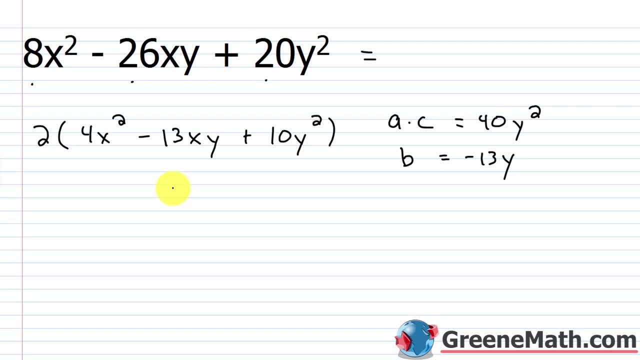 we know we have 1 times 40. That's obviously not going to work. 2 times 20 won't work, Not divisible 3.. 4 times 10 won't work. 5 times 8, we can make that work. If I had a negative 8 and a negative. 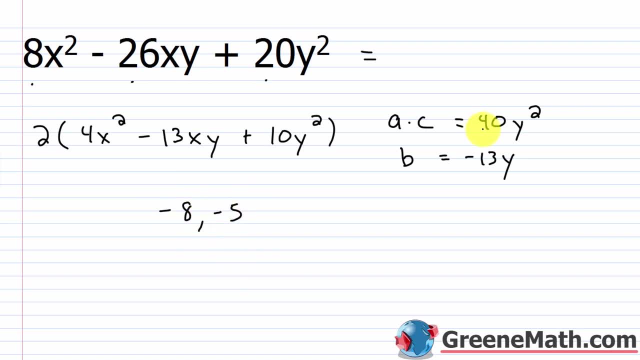 5, negative 8 times negative 5 is positive 40. Negative 8 plus negative 5 is negative 13.. And what I do is just attach a y to the end of each. So negative 8y and then negative 5y. 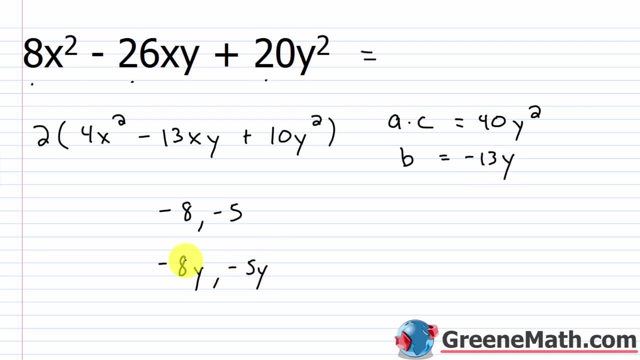 Because negative 8y plus negative 5y is negative 13y. Negative 8y times negative 5y is 40y, 40y squared. So it's not any more difficult when you have a second variable. You just kind of. 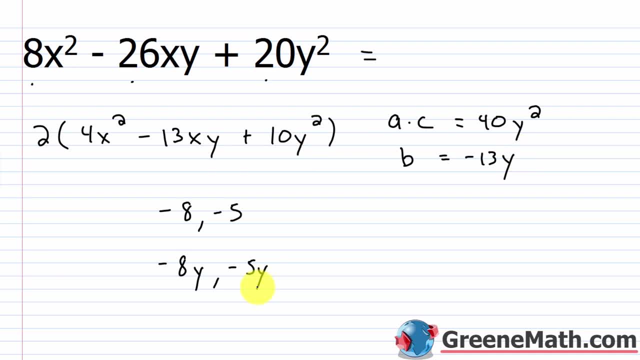 throw it in there, right, And it'll work itself out. Really, the only challenging part is finding the two integers. The variable is a breeze. So, knowing that this is what I have now, let me kind of erase this. I'm still going to rewrite my middle term. So I'm going to say: 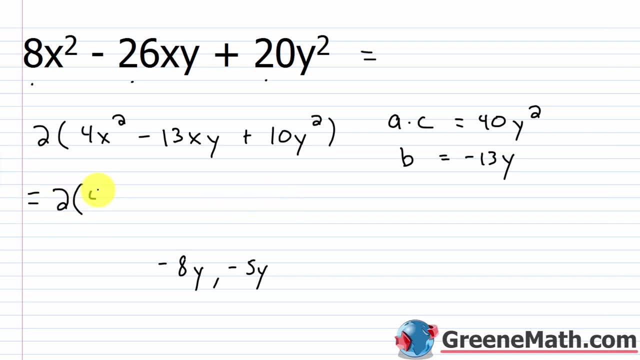 this is equal to, we'll have 2 times the quantity. You'll have 4x squared, Now the middle term, I have negative 13xy, So I'm going to use these two. I'm going to put minus 8 and then x, and then 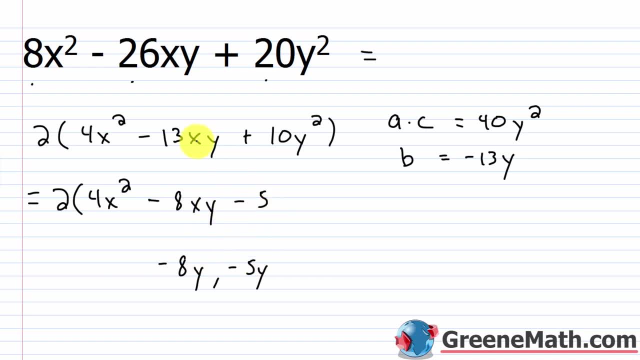 y And then minus 5, and then x and then y. So basically I just said: minus 8xy, minus 5xy. We know that would end up being negative 13xy. Then plus we have our 10y squared. 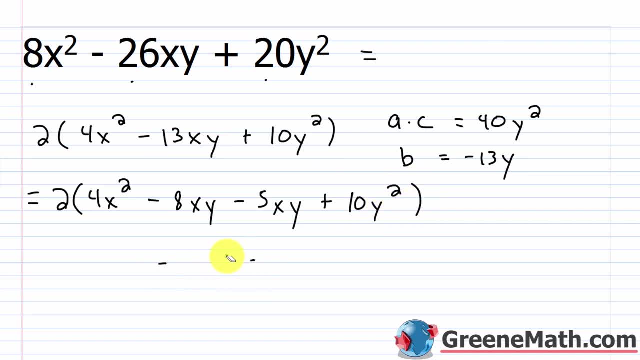 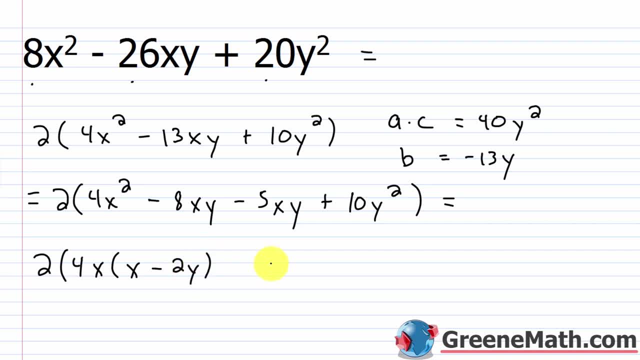 leave me with x minus 2y. In my second group I could pull out a negative 5y And that would leave me with x minus 2y. So I have a common binomial factor of x minus 2y And I'm just. 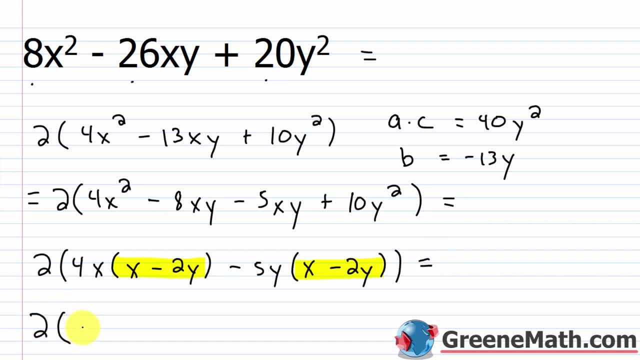 going to pull that guy out. So I'll have 2 times the quantity- We'll have x minus 2y- And then times the quantity 4x minus 5y. All right, let's take a look at another example with. 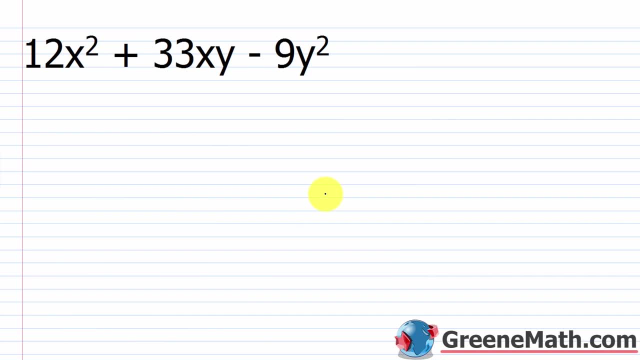 two variables involved. Let's say we saw something like 12x squared plus 33xy minus 9y squared. The first thing you'd notice is you could pull a 3 out before you begin, And this is very important to do this because it saves you work in the end. All right, you don't want to end up with. 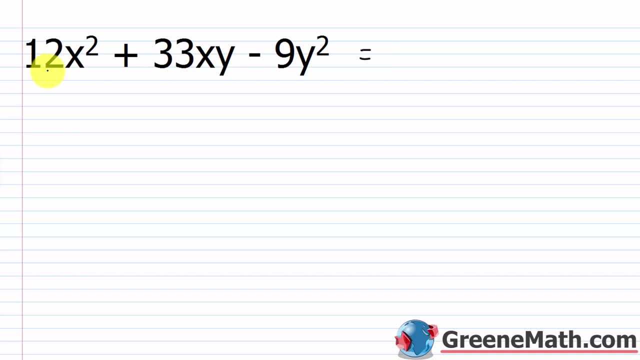 additional factoring because you might miss it All right. so if I pulled a 3 out, I'd have 4x squared plus 11xy minus 3y squared. Another thing that benefits you to pulling this out early is you're going to end up working with smaller numbers, Right, Smaller numbers are. 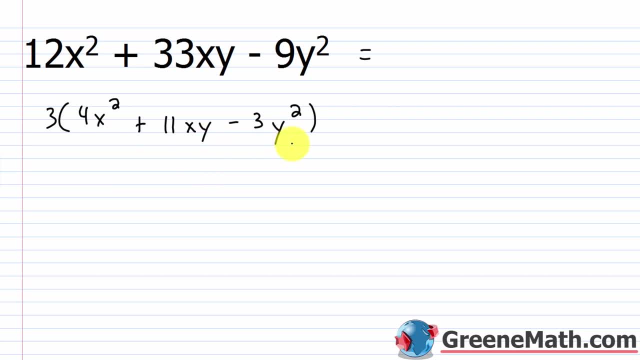 just easier to work with. So once I've done that again, I want to use the same process. Doesn't matter that there's two variables involved. I can label this as A, So I can say A is 4.. I can say B is what. 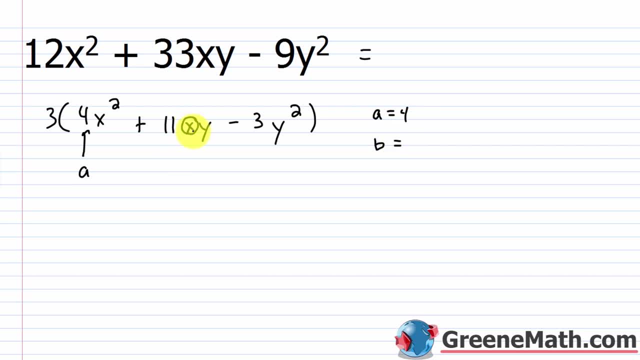 B is a numerator role, remember. it's the coefficient for x. so if x is being multiplied by 11 and by y, i could really say that b is 11y and then c is what it's. this whole thing here. it's this negative 3y squared. 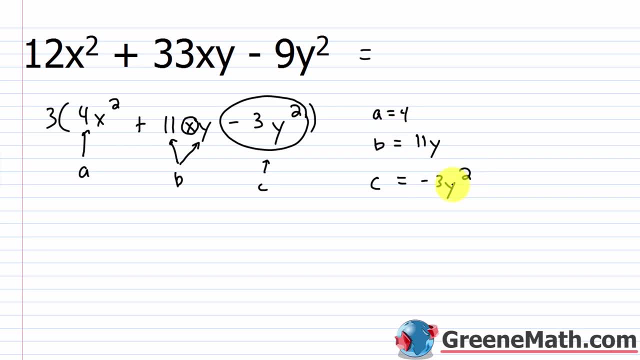 so if i want a times c, i would do 4 times negative, 3y squared. so ac is negative, 12 y squared and then b is 11y. but forget about these variable parts right here. this y squared and this y again if i work out the integers, in other words two integers whose product is negative, 12 and. 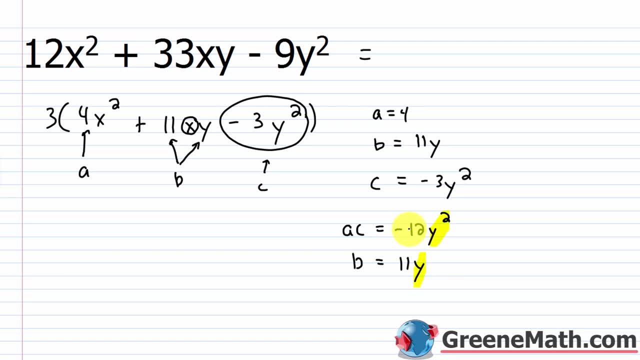 whose sum is 11, i can just tack a y on to the end of each and i'll have my answer. so if i want two integers whose product is negative, 12, i think about 12, i know i can do 1 times 12 and if i play, 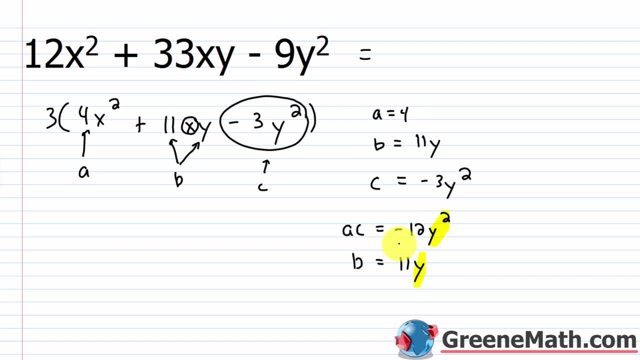 with the sine. if i do positive 12 and negative 1, that would work. so positive 12 again, put a y at the end, and negative 1 again put a y at the end. that's going to work. positive 12y minus 1y. 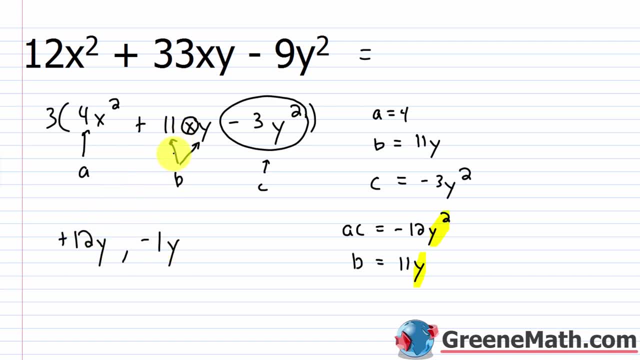 if i threw an x in the mix and i sum those two, i get 11xy. i'm going to use that to rewrite my middle term. so i'm going to have 3 times the quantity 4x squared and i'll do plus 12. don't just put plus 12y. remember this. you have an x involved there. so 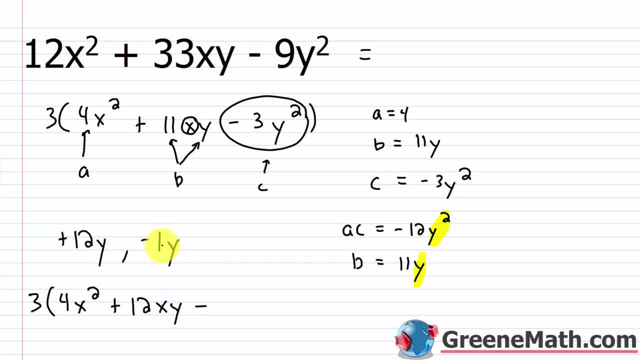 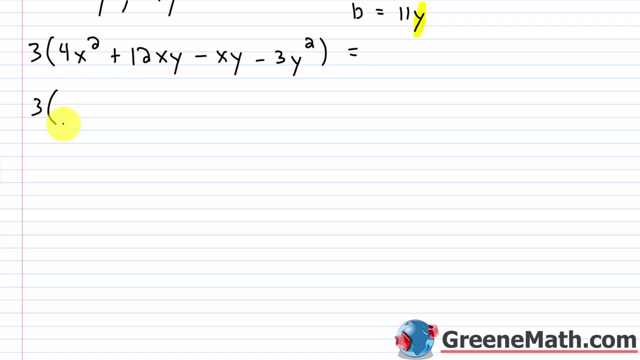 it has to be 12xy and then minus 1xy or minus xy and then minus 3y squared. let's scroll down, get a little room going. so factoring the inside here by grouping. we have three times inside of parentheses and the first group. i can pull out a 4x. so i pull that out. i'd have an x plus 3x. 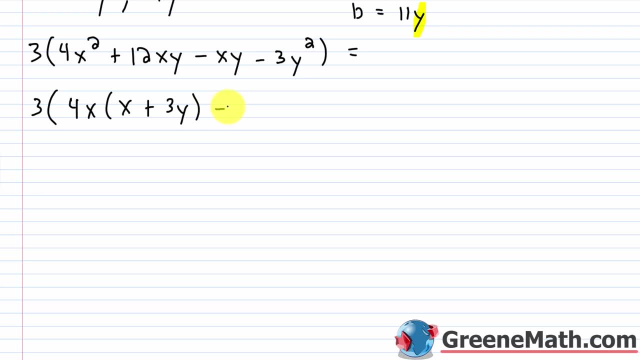 inside and the second group. i could pull out a negative y, so i'd be left with x plus 3y inside and again i get a common binomial factor of x plus 3y that i can pull out. so i'd have my three outside of parentheses and then i'd have x plus 3y. that quantity and then times i'd have 4x minus y. 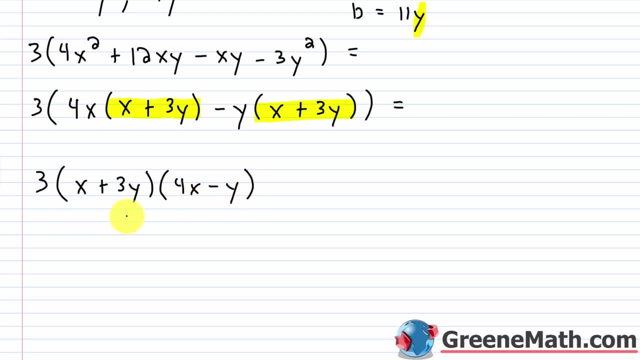 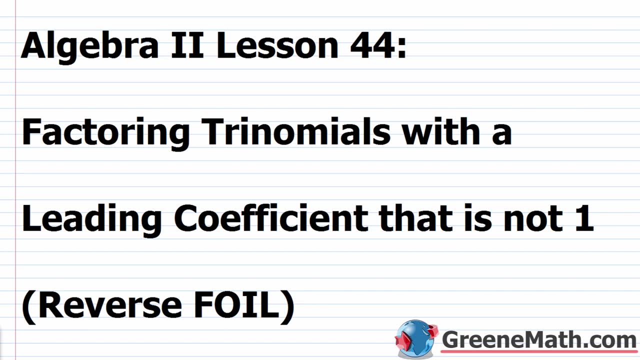 that quantity. so this is my answer: three times the quantity x plus 3y times the quantity 4x minus y. hello and welcome to algebra 2, lesson 44. in this video we're going to learn about factoring trinomials with a leading coefficient that is not 1, using the reverse 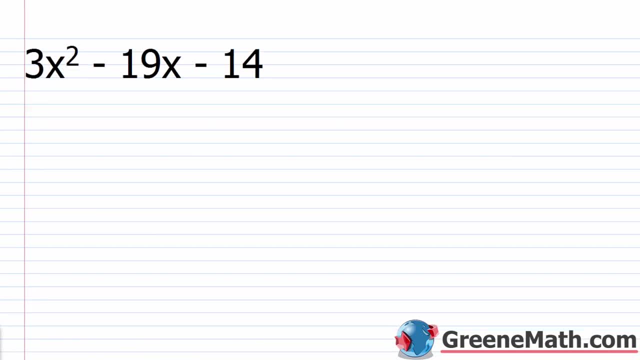 foil process. so again, for those of you who took algebra 1, you've seen this content before, so it's not too challenging for you, but you might just need a refresher on it. so how would we go about factoring this using reverse foil, if i say something like 3x squared minus 19x minus 4x? 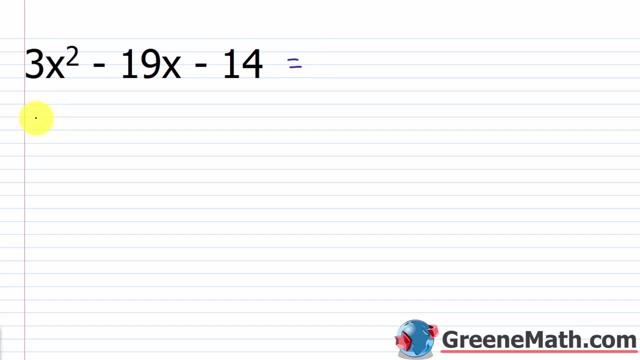 and i want to reverse the foil process. so i'm going to factor this into the product of two binomials and let's just write foil out for a second. so it's f for first terms, o for outer terms, i for inner terms and l for last terms. so the first thing you would think about is the fact: 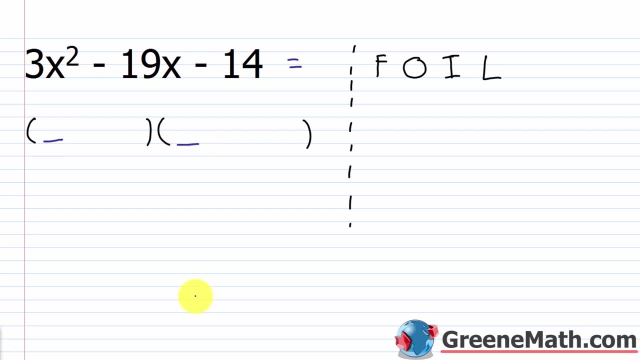 that this times this, okay, would give me this. now, this is a pretty easy scenario because the coefficient of x squared is a prime number, right three is only one times three, or if we're really thinking it could be negative one times negative three. but you don't want to put. 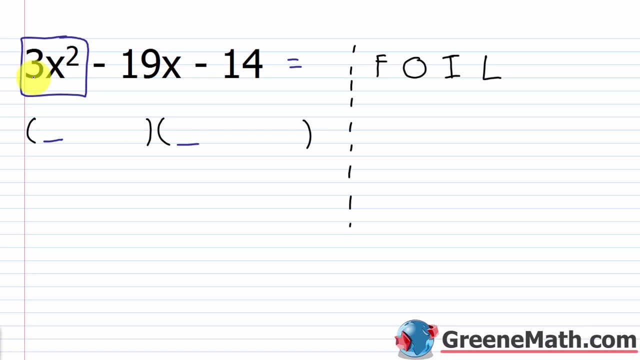 that there, because that would complicate things. okay, and i'll show you that at the very end: what would happen if you put negative one and negative three in. so i just think about three and one. okay, three and one. now i've got an x involved there, because it's x squared, so i would have three x. 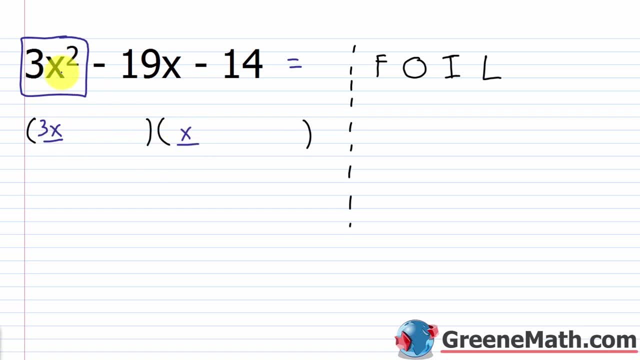 and then x. okay, three x times x is three x squared. so we've got that down and the order that i put this in wouldn't matter if i put my x here and my 3x over here. that's completely irrelevant. the next thing, okay, the next thing that you would think about is the fact that the last terms so this: 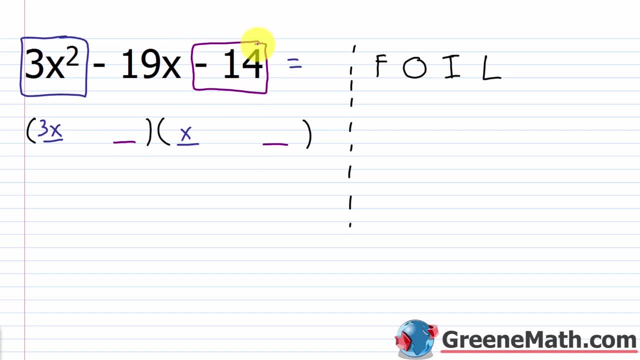 times this will have to give me this. it'll have to give me negative 14.. so i would think about factors of negative 14.. but it's got to be such that the outer and the inner are going to combine to give me that negative 19 x. 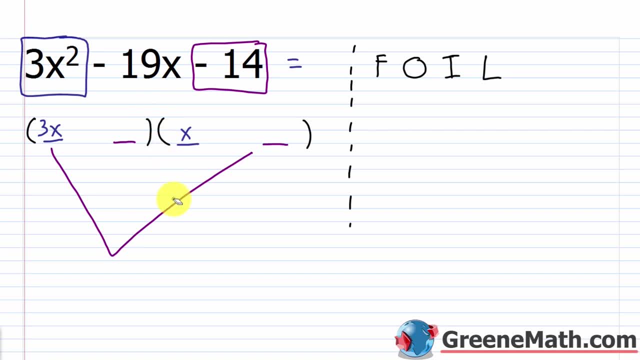 so that's where this trial and error is going to come in. i've got to go through all the possibilities. so, for negative 14, i've got to think about positive 1 times negative 14, and i've got to think about negative 1 times positive 14.. i've also got to think 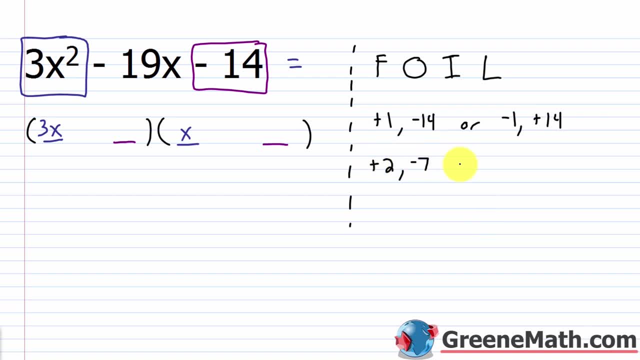 about positive 2 and negative 7, and then i've got to think about negative 2 and positive 7. okay, so more scenarios are involved. when you have something that's negative, because it's a negative times a positive, you've got to go back and forth between. 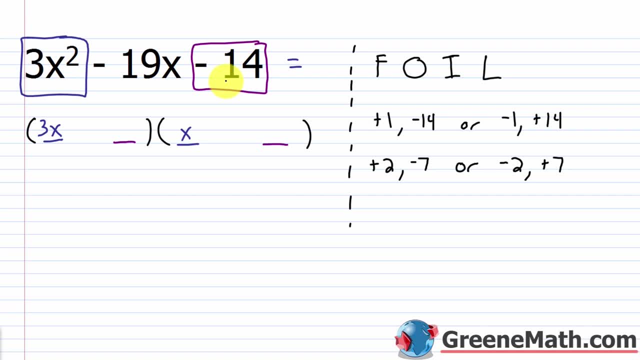 the possibilities. so the only thing we can really do is just go through and do trial and error. so in other words, i would set up some scenarios: so i have 3x, i have my x and let's just do another one down here. and sometimes i'll write out a bunch at once and just quickly go through the possibilities. 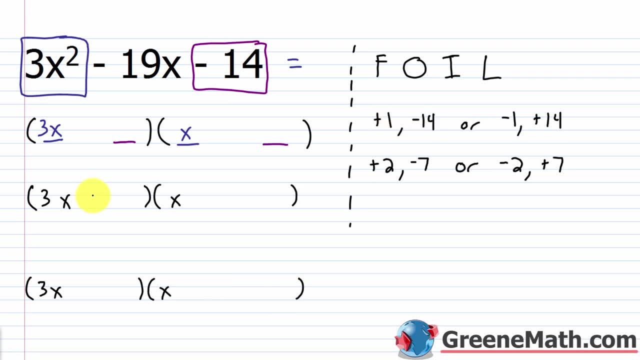 so let's start with this: positive 1 and negative 14.. so plus 1 here, minus 14 here, and then you've got to reverse that. so you're going to go minus 14 and plus 1 because you've got to check different. 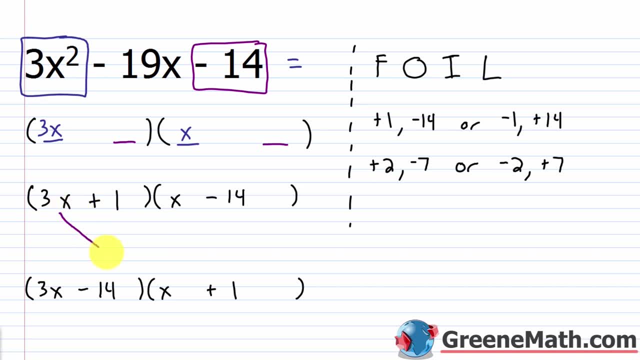 outer and inner products. in other words, for this one i'd have 3x times negative 14 and 1 times x. so same, dobrado, taking into account that, i'll just try to get a bigger thumbnail for you. in fact, i need to read a couple of other butterflies for my next project. 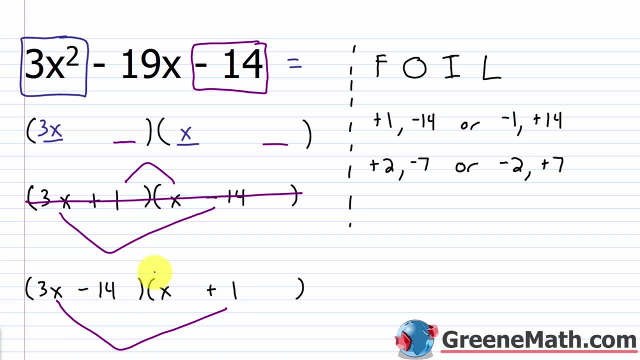 i'm going to have to correct this time. so let's take the right board, and i'm going to do the same thing here. i'm going to take the left off and then i'm going to have the right todas side per second, and then i'll have the expected to my学生 in terms of the 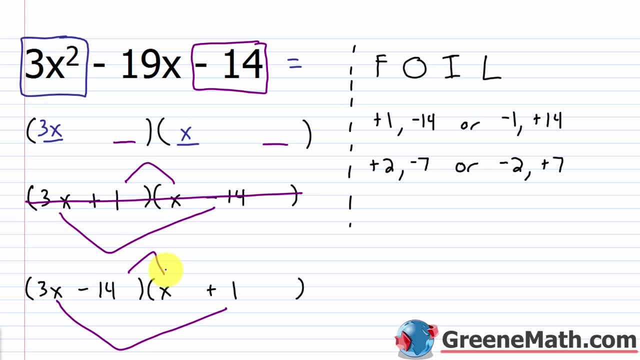 étape, and then i'm going to do the same thing, so i'll do the same thing again at the end. and then i have less than 6, so i'm going to do the same thing with eachición. so i'm going to write i Portal x to 3x times negative 14, so i'm going to put trx on it. 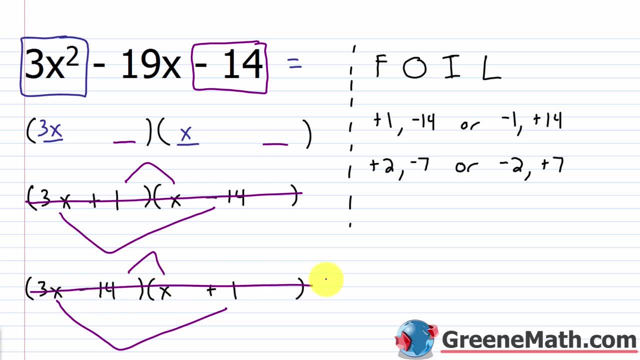 green Treasure soil bar, and that means negative 4x plus 1, so that's my 14, and So that's not going to work either. so you can line that out and say, well, positive 1 and negative 14 will not work. So then you go to the other scenario. so let me, let me erase this. and so in this scenario, 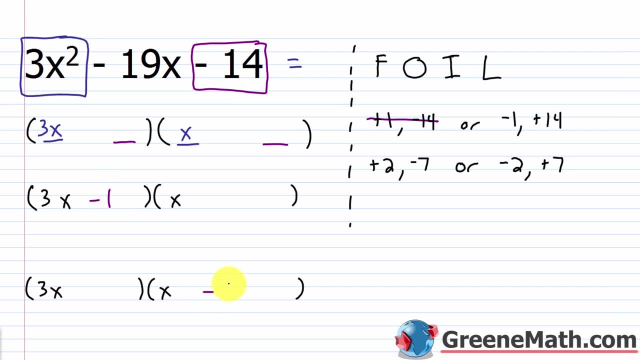 We have a negative 1, so I'll put a negative 1 here and here and a positive 14, so I'll put that here and here. So what am I checking? so 3x times 14 will be 42 X and the negative 1 times X would be negative X. 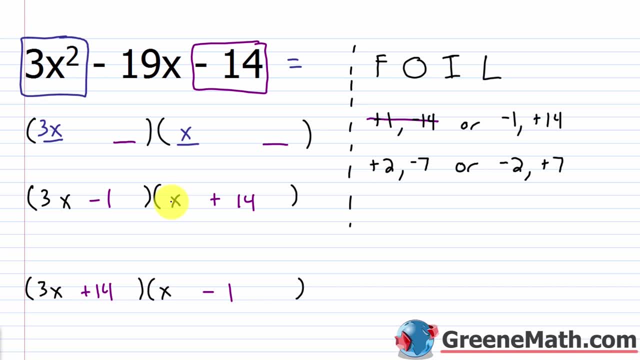 So 42 X minus X is 41 X. so that won't work for this one. 3x times negative 1 would be negative. 3x 14 times X would be 14 X. so 14 X minus 3 X would be 11 X. so this is gone. 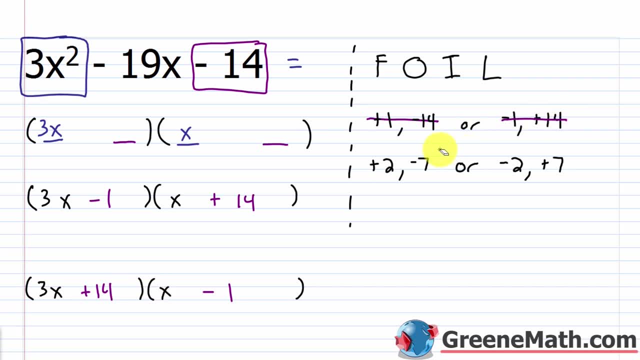 That's no longer a possibility. we can move on to the other scenarios. Now, when we get to this scenario, here again we have positive 2 and negative 7. so plus 2 negative 7, negative 7 plus 2. All right, so let's check this one. So 3x times negative 7 is negative 21, X. 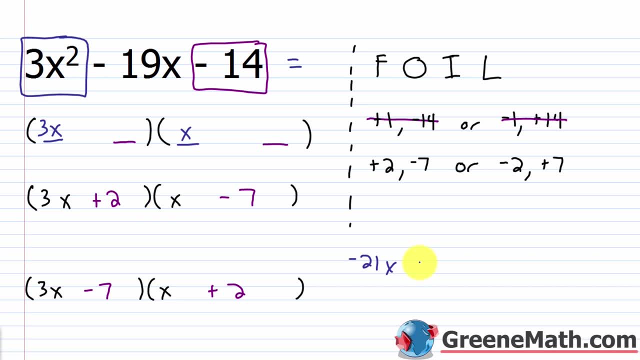 and then 2 times X is positive 2 X and That would work. Negative 21 X plus 2 X would give me negative 19 X. 2 times negative 7 is negative 14. So this is your correct factorization. Let me erase all this. I don't need to try anything else. 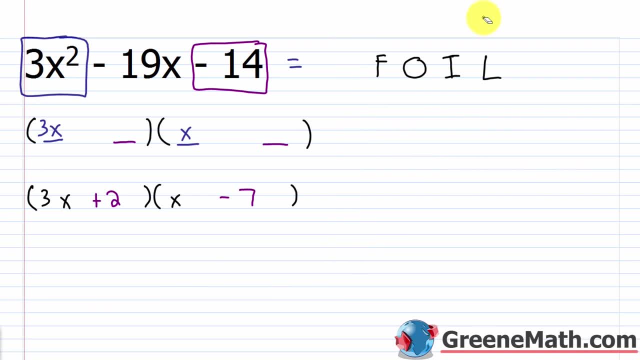 And sometimes you hit it right away, Other times it takes you a while. But this is our correct factorization and if you want, you can use foil and check it 3x times X is 3x squared, Then the outer 3x times negative. 7 is negative, 21 X. 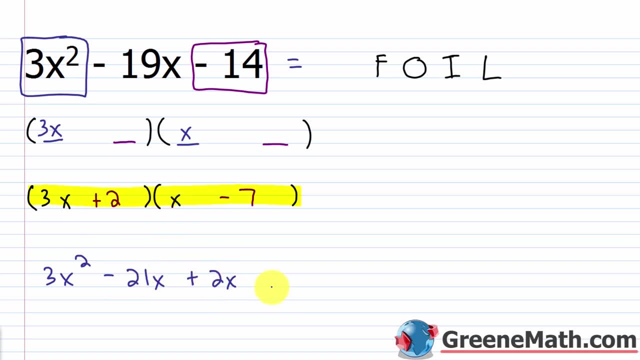 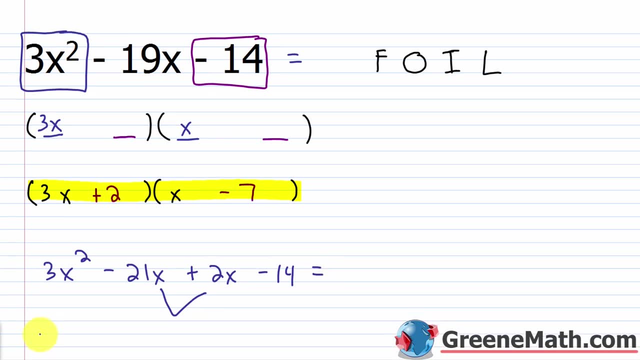 Then the inner 2 times X is positive 2 X, Then the last 2 times negative 7 is minus 14. if I combine like terms here in the middle, I'm gonna end up with 3x squared minus 19, X minus 14. that's exactly. 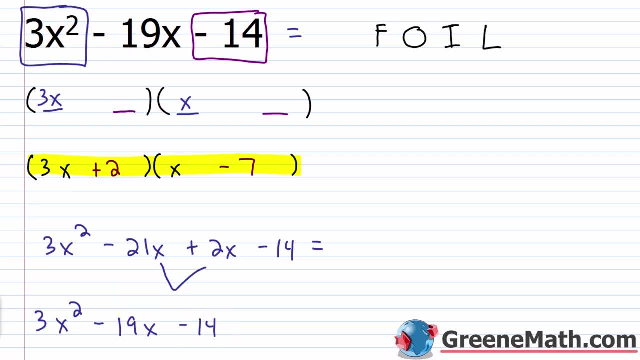 What I started with right there. now let me give you a little insight into why We wouldn't want to say: start out with negative 3x and negative X. I can factor out a negative 1 from this. if I wanted to, I could say this is negative 1 times and I can make this negative. 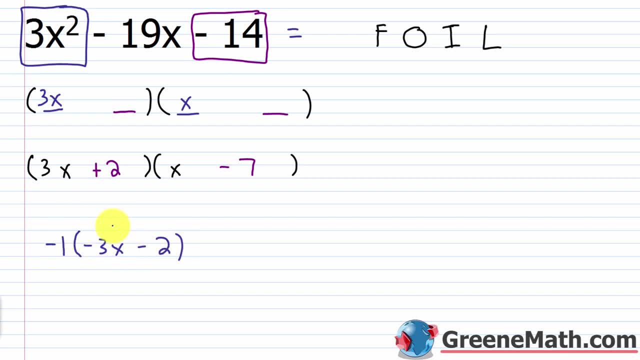 3x and this minus 2. I just pulled a negative 1 out. I'm legally allowed to do that. then times: I could pull a negative 1 out from here as well. negative 1 times: you'd have negative X plus 7. This is mathematically the same as this: 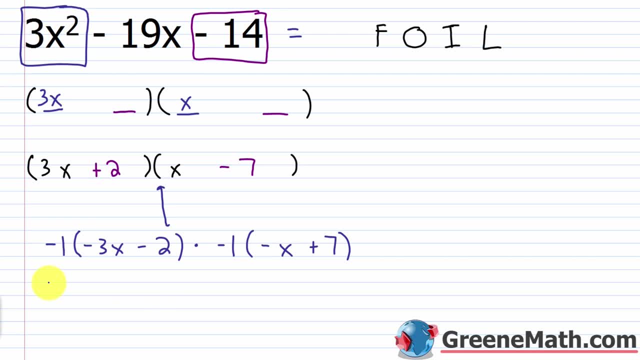 Negative 1 times negative 1 is 1, so really I could write this as negative 3x minus 2, that quantity times negative X plus 7. So I could have began, if I wanted to, with the negative 3x and negative X. so when you see something positive that's leading, you can do this if you want. but 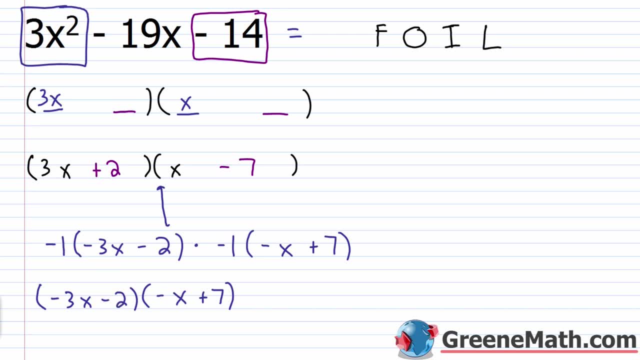 Working with negatives in the leading position makes it a little bit more complex. You want to make things as easy as you can make them, So it's just better to start out with a positive here and a positive here. If this is positive, you know you can make that work because of what I just showed you. 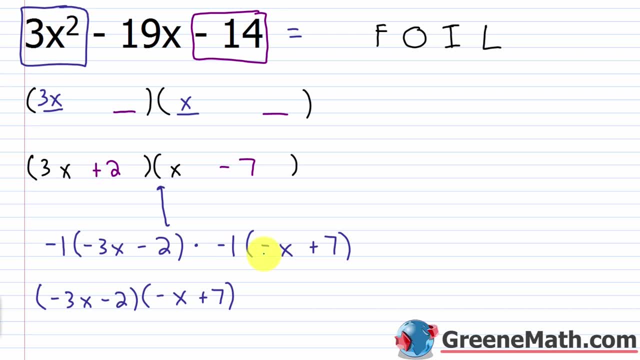 You can always factor out a negative one from each of those. multiply the two negative ones together and get one. One times, anything is just itself. And just to completely prove this to you, because I know some of you are like no, that. 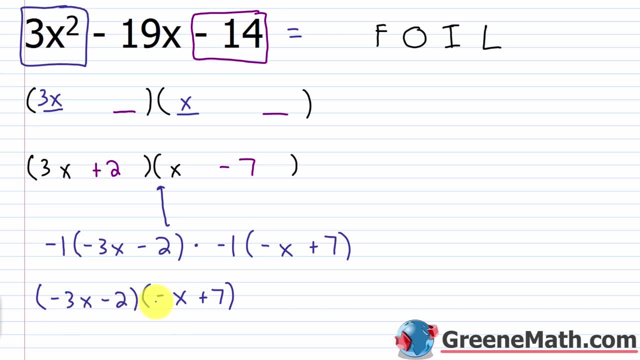 doesn't seem right. If you do FOIL on this. negative 3x times negative, x is what That's: 3x squared. Negative times negative is positive. 3 times 1 is 3, x times x is x squared. 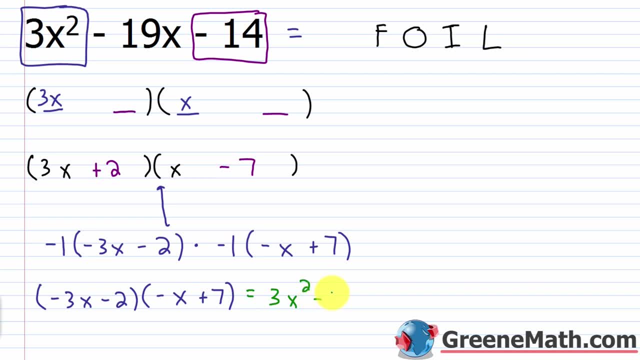 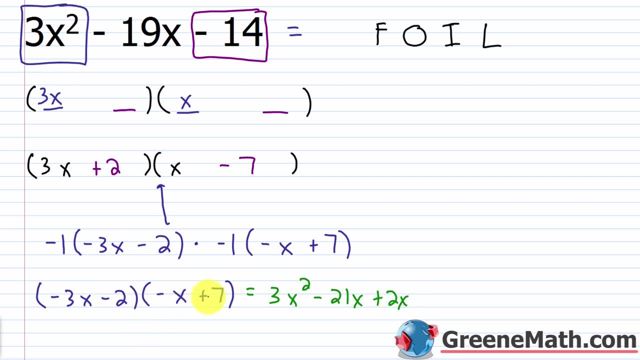 The outer negative 3x times positive. 7 is negative 21x. then my inner negative 2 times negative. x is positive 2x. then my last negative 2 times positive. 7 is negative 14.. So if you combine like terms in the middle again you would get 3x squared. 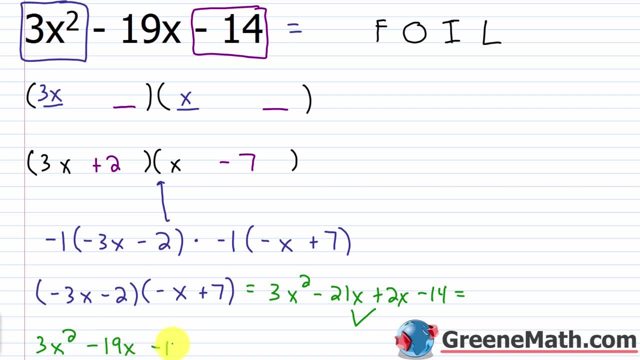 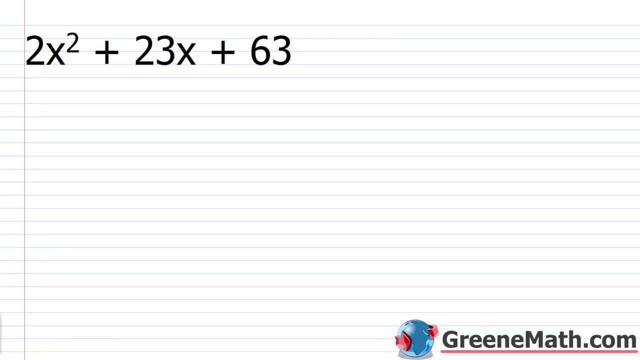 Minus 19x, minus 14.. So again, that's why I just started out with this, because it's going to be the same as this. Okay, And it's just easier to work with positives in the leading position. All right, let's look at another one now. 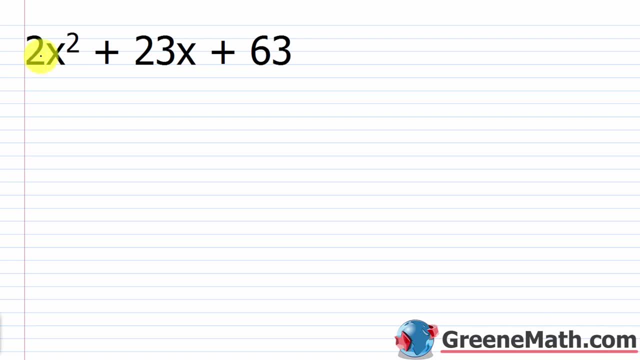 And we did our first one, so it should go a little bit quicker. So we have 2x squared plus 23x plus 63.. All right, so we're going to factor this into the product of two binomials Now. 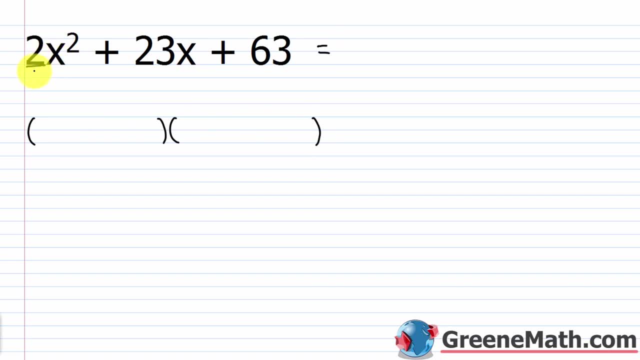 So my coefficient for the leading term here is a 2. That's a prime number. so again, that's a very easy scenario because I know 2 is just 2 times 1.. And again, for the reasons that I just covered, I don't want to think about negative 2 and 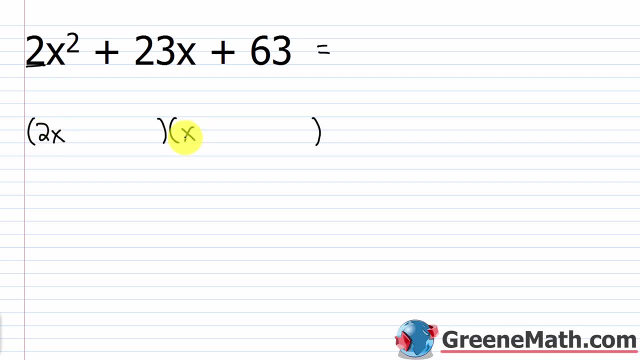 negative 1.. So I'm just going to go 2x times x and be done with that. Now I just need to think about 63 here. What are the factors of 63?? So what times? what would give me 63, but then, through the process of combining like terms, 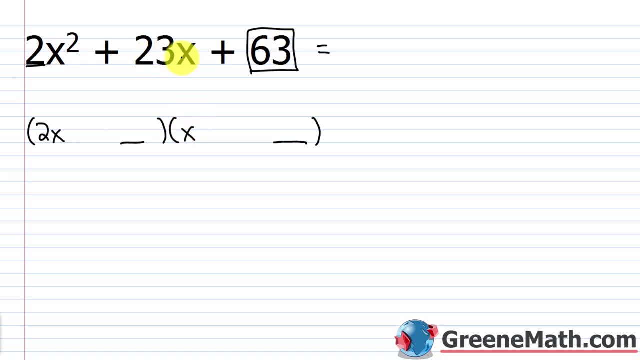 with the outer and the inner. we would want to get a 23x in the middle, And for this everything's positive. So I'm just going to think about positive numbers here. So 1 times 63, it's not divisible by 2, it is divisible by 3.. 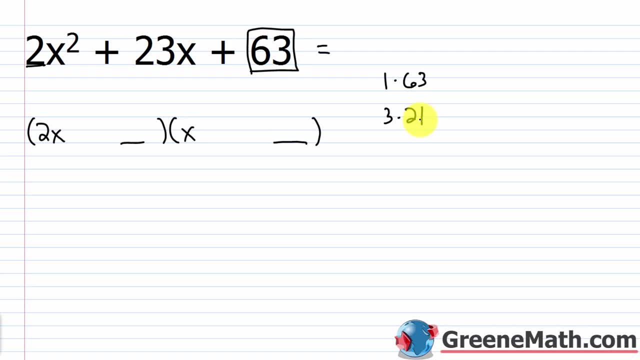 So 3 times 21,, not divisible by 4,, not divisible by 5, is divisible by 7,, 7 times 9, and that's all we're going to get. So lots of possibilities here If you think about this. this right here is very far apart if you think about the numbers. 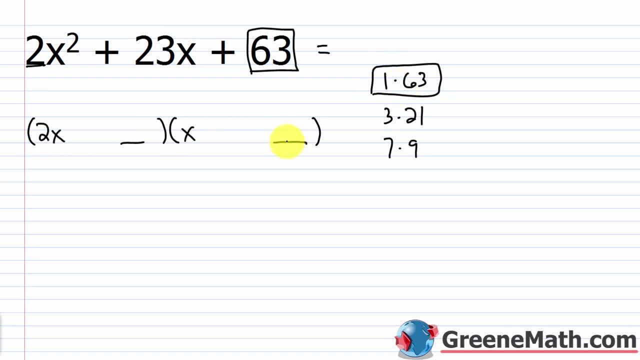 1 and 63 are far apart. If I was multiplying 2 times 63,, I'd have a really big number. Or if I was just multiplying 63 times 1,, I'd have 63.. This one isn't going to work. 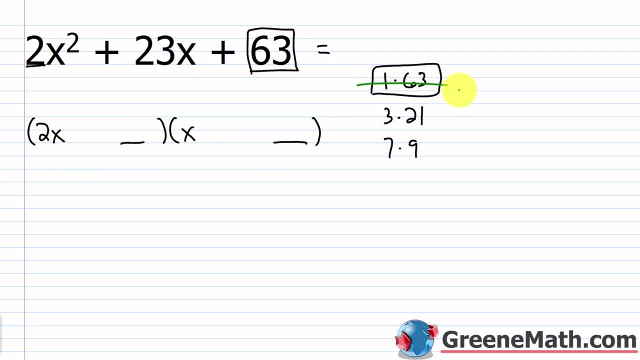 You can eyeball that and see that you can just eliminate that right away Now. 3 and 21,. I might be able to get that to work. I just have to check the different possibilities. So 2x x, so 3 and 21.. 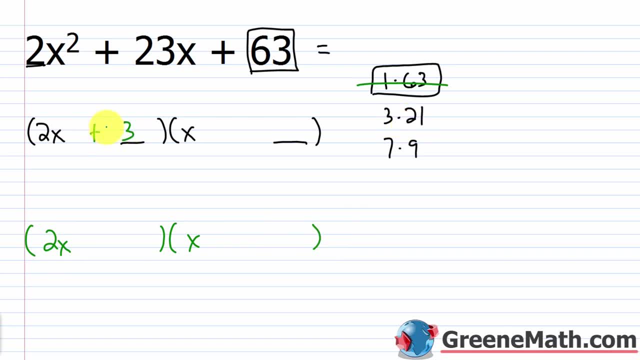 So I'm only going to check 3. Positive, 3. Positive 3. Positive 3 here and positive 21 here. and because I'm only using plus signs here, it's much quicker. The other scenario is positive 21 here and positive 3 here. 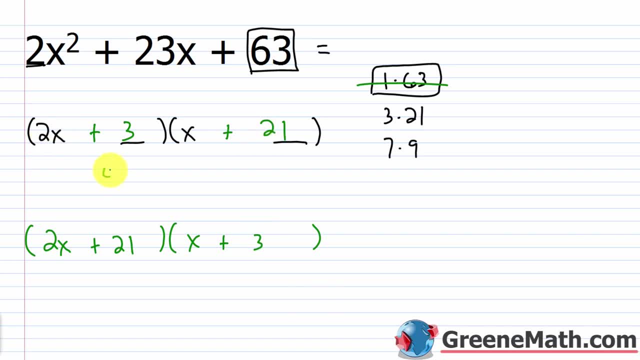 So check your outer and inner 2x times 21 would be 42x. 3 times x would be positive 3x. this would combine to be 45x. so this isn't a possibility. You can line that up. 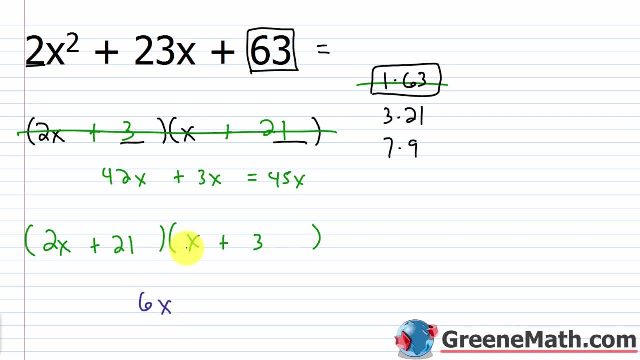 For this one, 2x times 3 would be 6x, and then 21 times x would be 21x, So that would be 27x if we added. so that's not a possibility either. We can line this out. 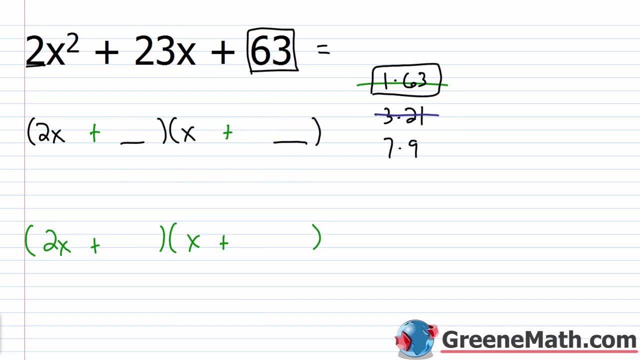 So now our last possibility is to use 7 and 9.. So I would do 7 here and 7 here, 9 here and 9 here. So the outer 2x times 9 would be 18x, and then 7 times x would be 7x. 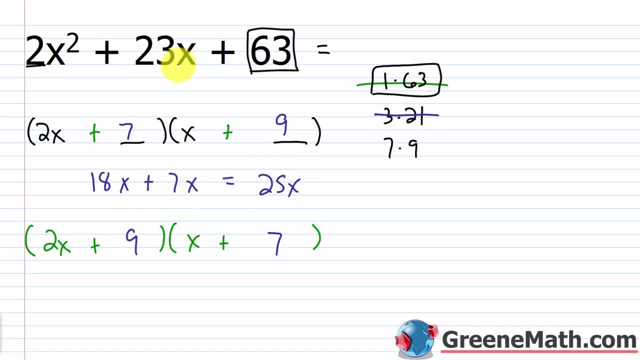 If you add those together you get 25x, That's not 23x. so this is eliminated. So it has to be this possibility, or it would be prime. So 2x times 7 would be 14x, and then 9 times x would be 9x, and if we combine 14x and 9x, 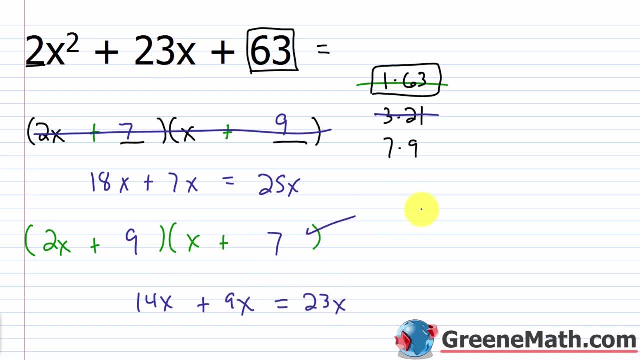 we do get 23x, So we do get that. so this is the big winner. Let me erase everything, And again you can check this through: FOIL 2x times x is 2x squared. The outer 2x times 7 would be 14x. 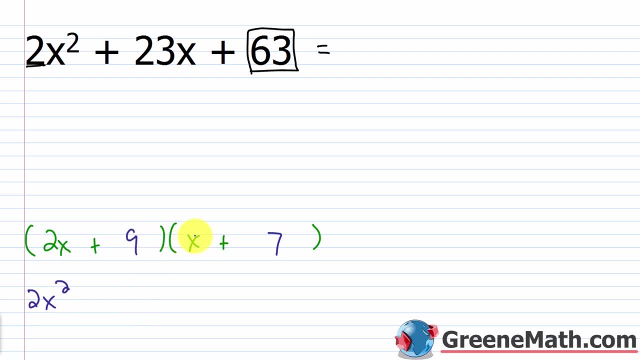 The inner 9 times x would be 9x, 14x would be 9x, 14x plus 9x would be 23x. so plus 23x, And then 9 times 7 would be 63.. 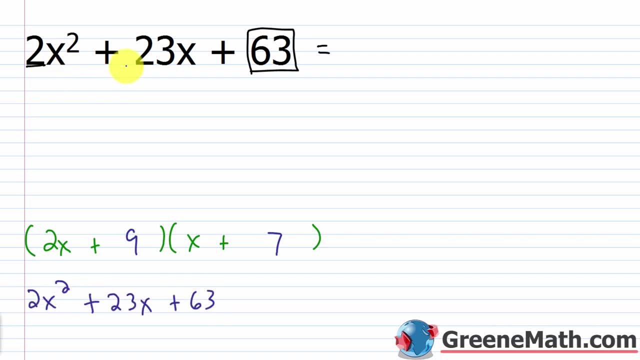 So you can see, you got exactly what you started with 2x squared plus 23x plus 63.. All right, let's look at a few more. I think for most of you you've kind of figured this out by now. 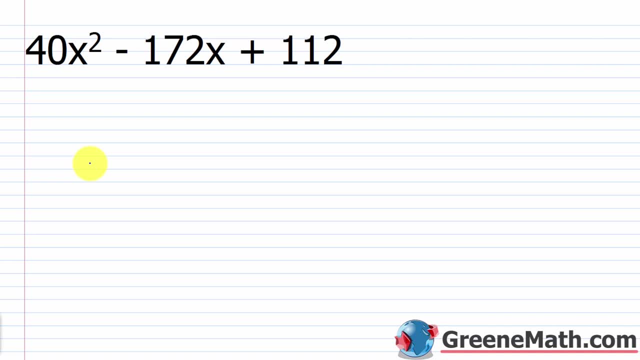 We're gonna look at one where the leading coefficient is not a prime number. It makes it more tedious, not any more difficult. So 40x squared minus 172x plus 112 is what we're gonna try. So we got a little bit of a long list here. So what we're gonna do here is we're gonna do a little bit of the other ones, But first we got a little bit of a problem here. Let's do a little bit of the other one. So what we're gonna do here is we're gonna do a little bit of the other ones. 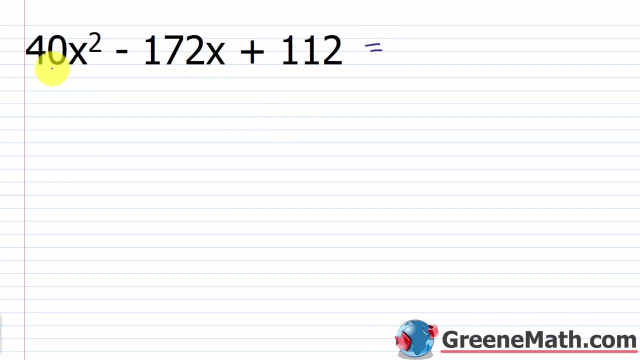 is what we're gonna try to factor. Obviously, if you look, everything's even right. I've got a zero, a two and a two. But if you further think about this, you should know that 40 is divisible by four. 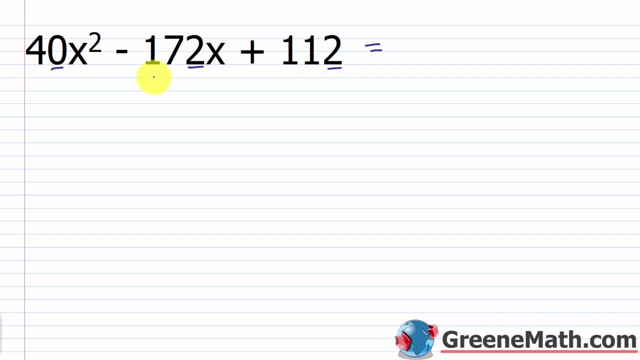 and 112 is divisible by four. Those are obvious For 172, forget about the negative for a second. for 172, well, 72 is divisible by four. so I know 172 is. So that means I can pull a four out before I even start. 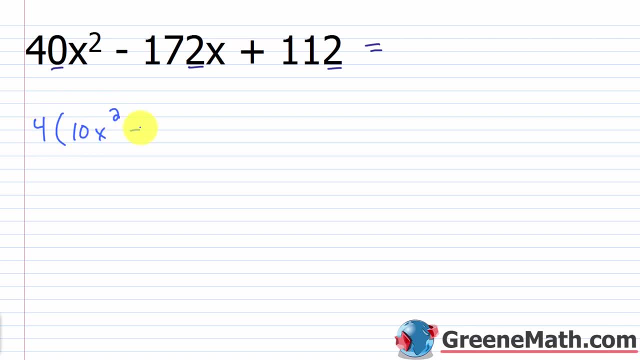 So if I pull a four out, I'm gonna have 10x squared minus 43x plus 28.. All right, so I wanna factor the inside of this now, So we'll have four times inside of my parentheses. Now, if I have 10x squared, 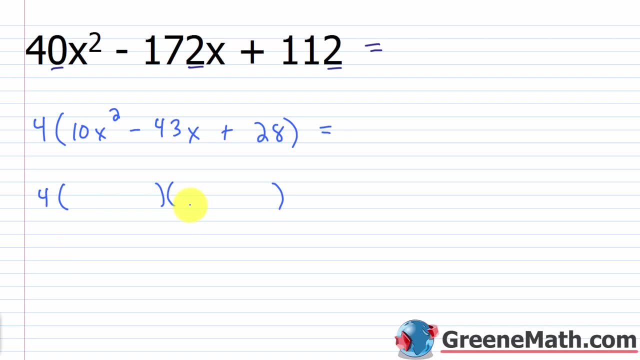 it is not obvious what's gonna go here and here 10 is not a prime number. The factors of 10 are one times 10 and five times two. And again I know you could do negative one times negative 10 or negative five times negative two. 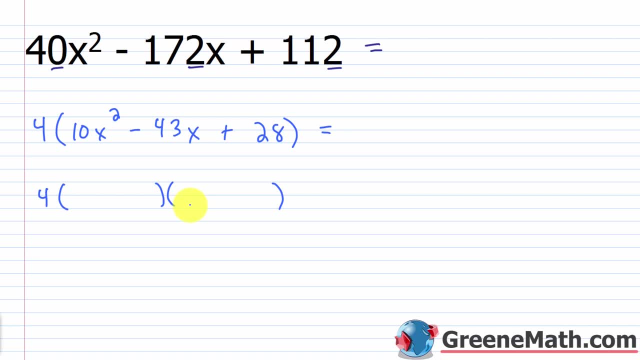 but we don't need to think about that again for reasons that we already covered. So I've gotta go through and try as different scenarios- five x times two x or the other scenario I would have is four times a quantity. 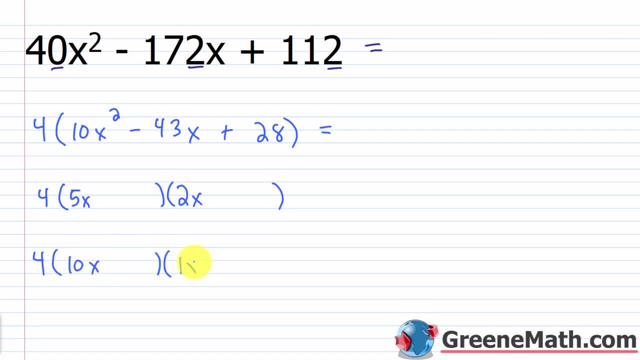 You'd have 10x and then times one x or just x. So these are what we're gonna consider here. It becomes more complex because the final term is positive and the middle term is negative. So what does that tell me? It tells me that, to get this, 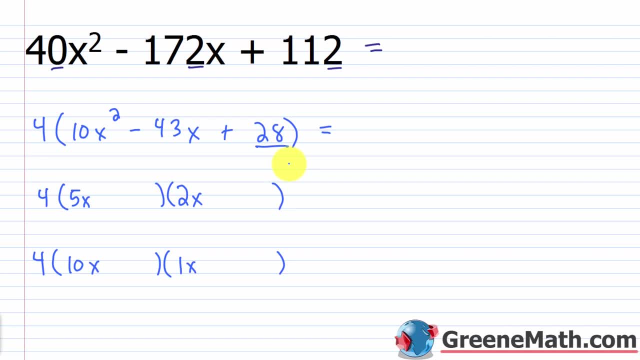 I had to have a negative times, another negative. So that tells me that these positions here are going to be negative values. So what are the factors of 28, considering only the negative values? Well, I know it's one times 28.. So that would be. let me kind of just make a line here. 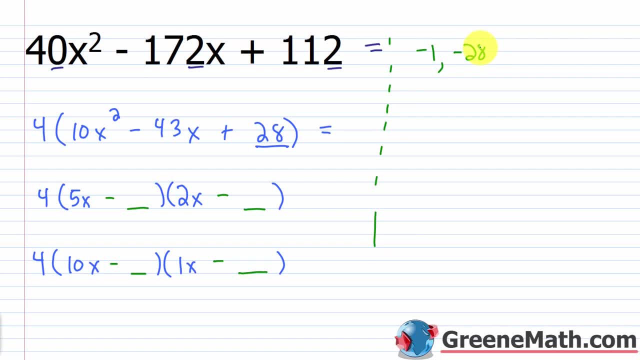 Negative one times negative 28.. I know it's two times 14.. So negative two times negative 14.. I know it's four and seven. So we think about negative four and negative seven, And so that's all we're gonna have. 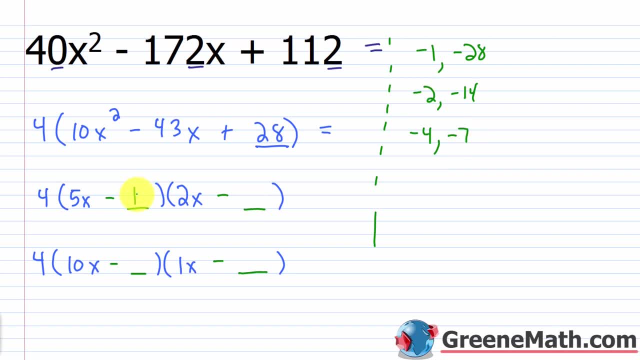 So let's start out with a scenario where I have negative one here and I have negative 28 here. Now, one thing that I haven't told you, and I've talked about this in algebra one: if there's not a common factor in what you're trying to factor, 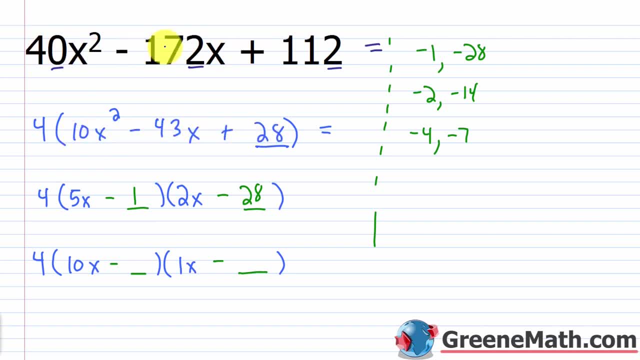 So, in other words, we're trying to factor this, Forget about this, Say oh, there was a common factor of four. That doesn't matter, We've already pulled that out. If there's not a common factor here, then none of the factors for this. 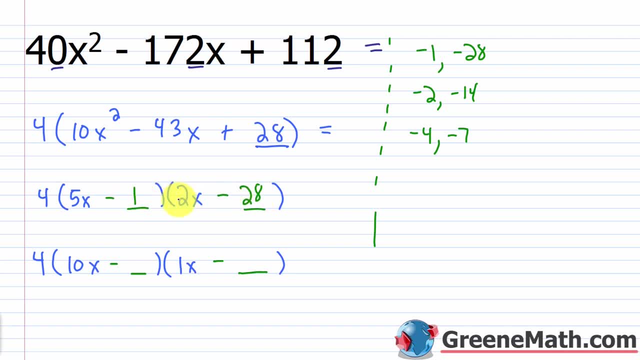 meaning neither of these binomials would have a common factor. Two and 28 have a common factor of two, So this isn't a possibility. I can try the other alternative for this, which is if I have a 28 here and a one here. 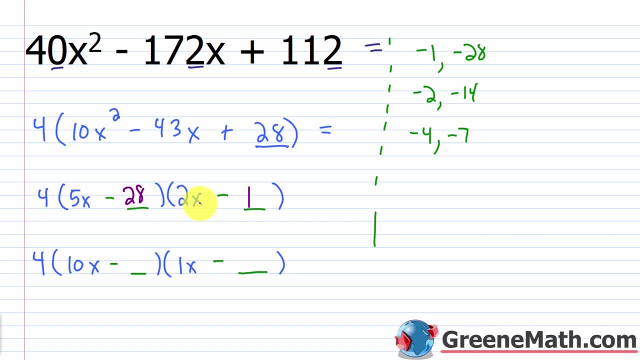 So four times the quantity five X minus 28 times the quantity two X minus one. That's a possibility, but you'll see that we're going to rule this out right away, because the outer five X times negative one is negative five X and the inner negative 28 times two X is negative 56 X. 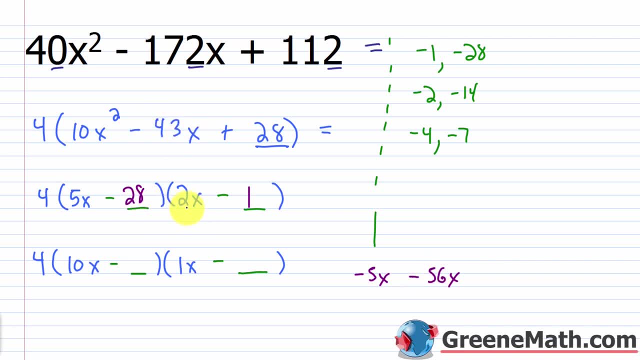 Those two are not going to combine to give me negative 43 X, So that is not a possibility here. Now let's erase that And I'm going to move on to the next scenario, which is negative two and negative 14.. Now 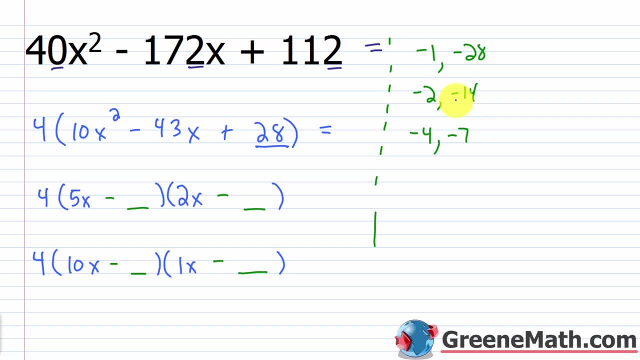 we can eliminate that right away. And why can we eliminate that right away? Well, if I put a negative two here and a negative 14 here, I've got a common factor of two. If I switch the order of that and I put a negative 14 here and a negative two here, 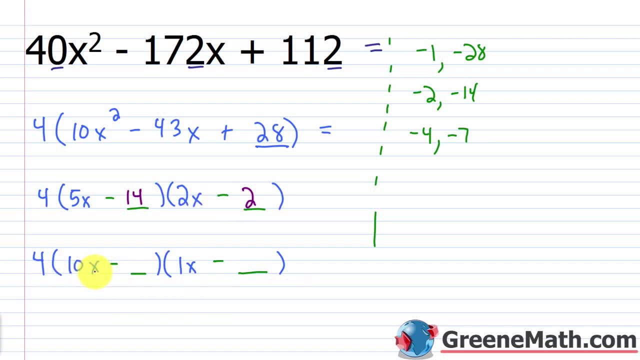 still got a common factor of two. And it's going to be the same thing when I get down to this. if I need to, If I put 14 here and two here, common factor of two. If I put two here and 14 here, common factor of two. 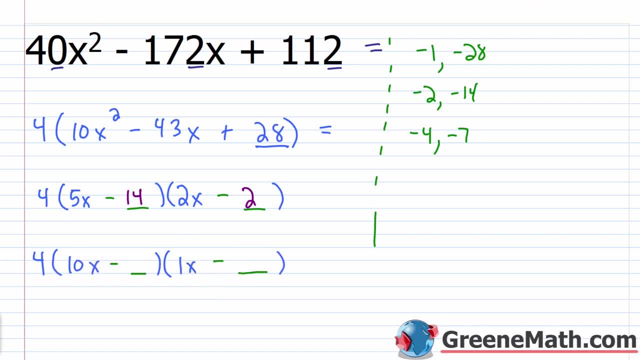 So either way you do that in any scenario, this is eliminated. You don't need to worry about that. Now I want to check this one right here in this, And if that doesn't work, we're going to move on to this scenario. 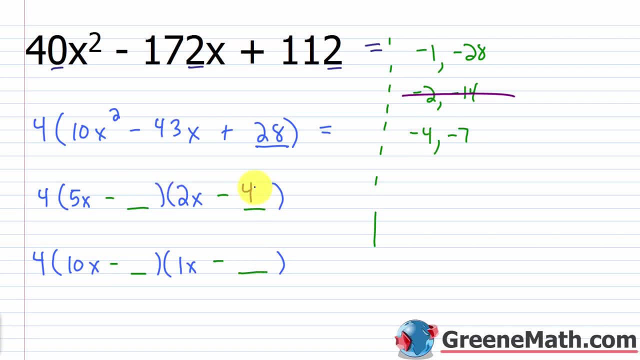 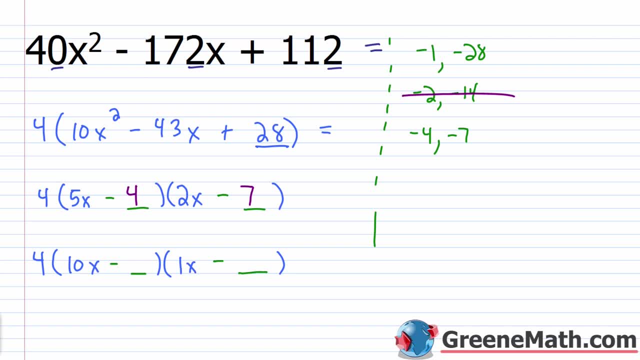 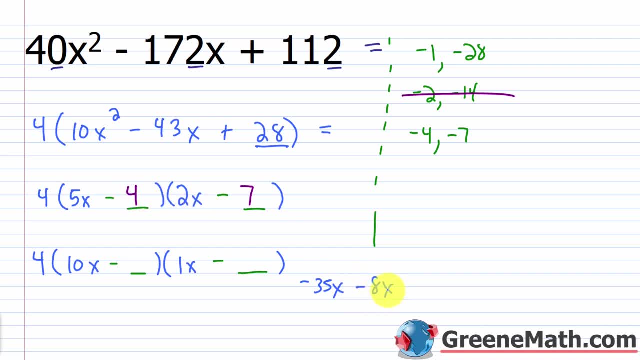 And then I would have negative four times two X, which would be negative eight X. So it looks like that's the big winner. Negative 35 X minus eight X is negative 43 X. Right, that's what we want, right there? 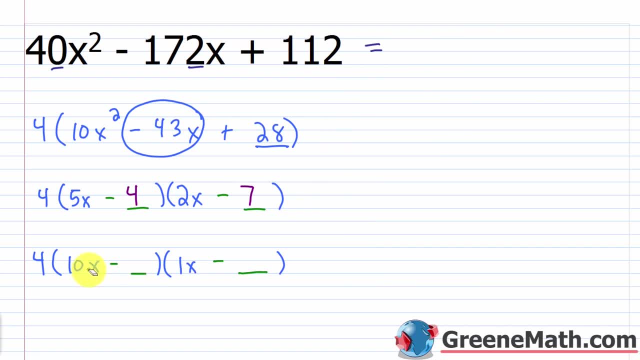 All right, so let's erase everything. And we're lucky because we didn't have to go into this scenario at all. All right, so we found the correct factorization. All right, so we found the correct factorization. All right, so we found the correct factorization. 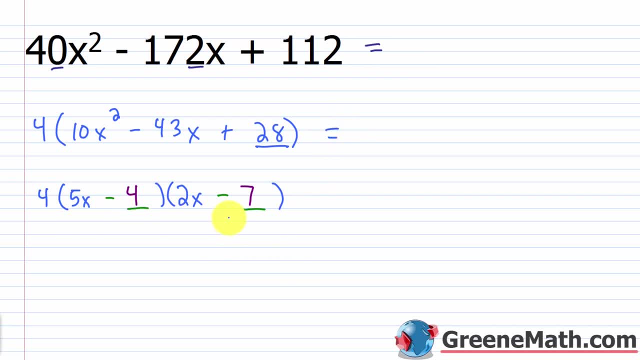 If you want to, you can go ahead and check this. You could do five X times two X. that would give you 10 X squared. The outer five X times negative seven would be minus 35 X. The inner negative four times two X would be minus eight X. 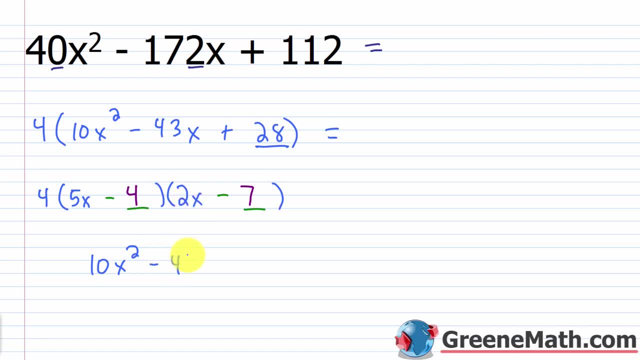 Negative 35 X minus eight X would be negative 43 X. And then the last negative, four times negative seven, is positive 28.. So that gives you this, and you're multiplying this by four. And when you multiply it by four, four times 10 X squared, would give you 40 X squared. 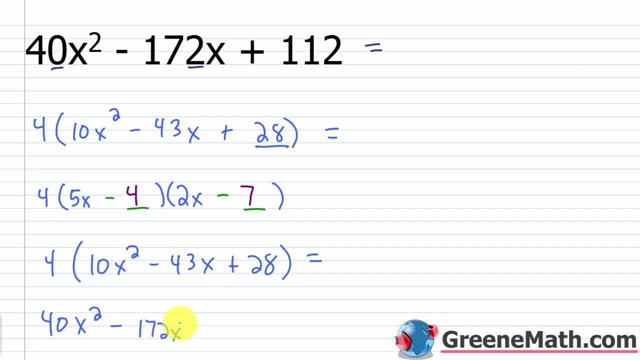 Four times negative 43, X would be minus 172 X, And then four times 28 would be positive 112.. So you get exactly back to this. All right, let's take a look at one final problem, And I gave you one here that has two variables involved. 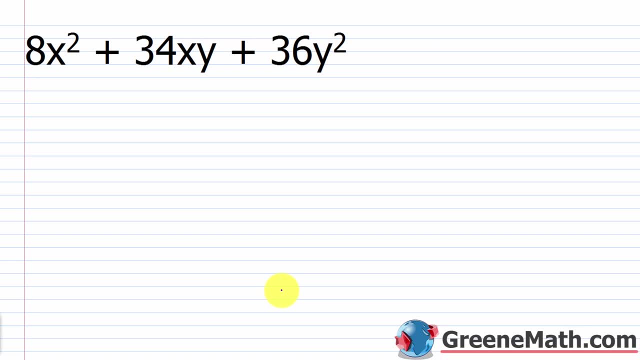 You've seen factoring with this before. You know at this point that it's not any more challenging. Right, You can almost just ignore the second variable, work everything out and then come back to it. So if I have eight X squared plus 34 X Y plus 36 Y squared, 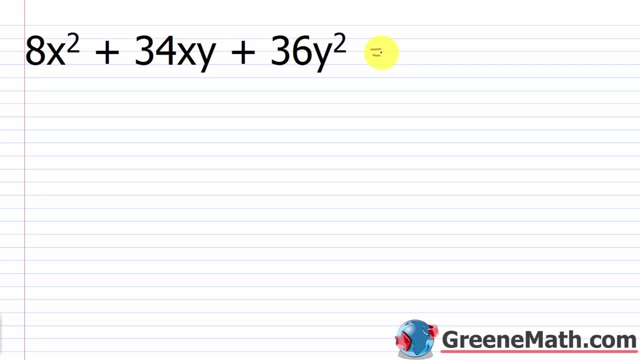 the first thing you would notice is that what Everything is divisible by two. So I could pull that out before I even begin. So if I pull out a two, I'd have four X squared plus 17 X Y plus 18 Y squared. 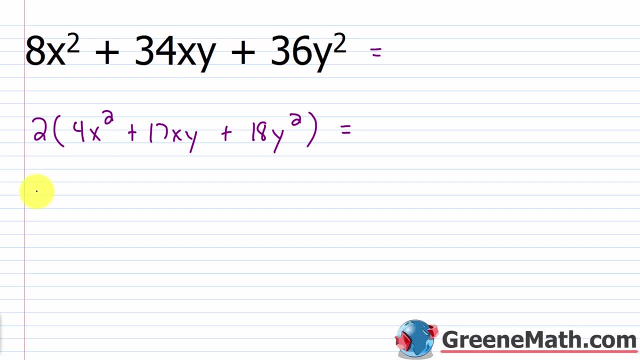 And so once that's done, we want to factor this, inside of parentheses, into the product of two binomials, So I think about four X squared. I know that can come from what It could come from: four X times X, or it could come from two X times two X. 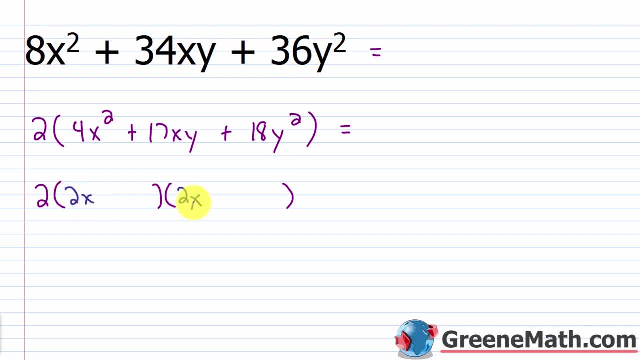 So we've got kind of two scenarios here And again we're not gonna think about the negative version: negative two X times negative two X, or negative four X times negative X, for the reason we talked about earlier. All right, so let's do this one. 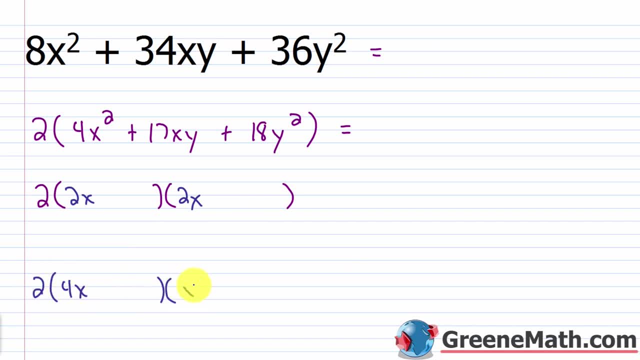 or you'd also have this one Now, once we've worked this part out, I know that Y times Y gives me Y squared. You can just throw this in and forget about it, okay, We know that from working previous problems. Y times Y is Y squared. 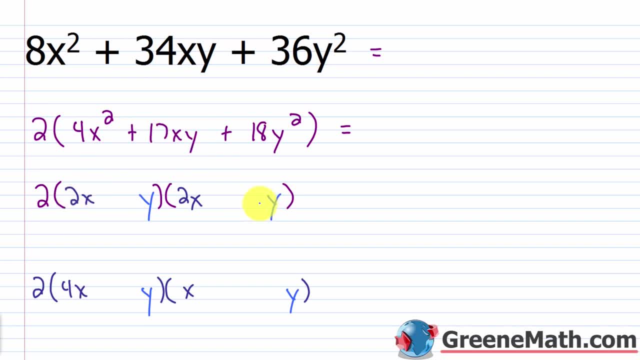 When you do your outer, you get X- Y as a variable. When you do your inner, you get X- Y as a variable. So when you combine like terms, you're gonna have a term with X- Y. So just put your Y in there. 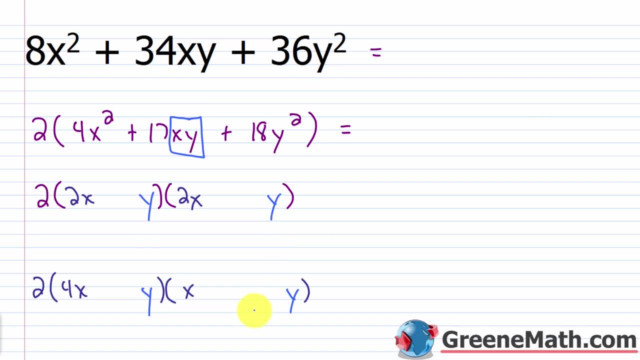 or whatever your second variable is, and forget about it. Don't stress about having two variables. It's super, super simple. All right, so the next thing is to work things out. You know that you're just gonna focus on this. 18 here. 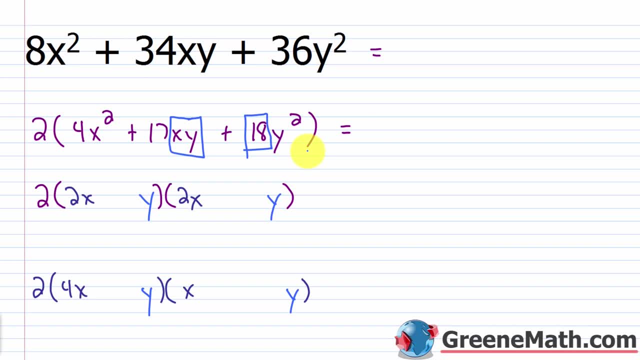 And everything's positive. so I'm just gonna focus on positives. And so I would have what For 18, one and 18, two and nine, and then three and six. Now I've gotta go through many possibilities here. 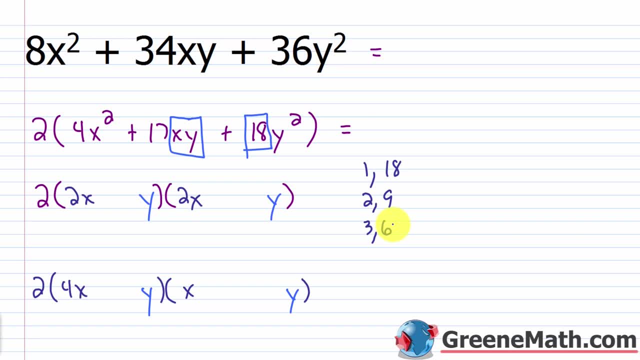 So let's think about for a second what we can eliminate right away For one and 18, it would not work in here at all Because I'd have to put an 18 in here somewhere and it would have a common factor of two. 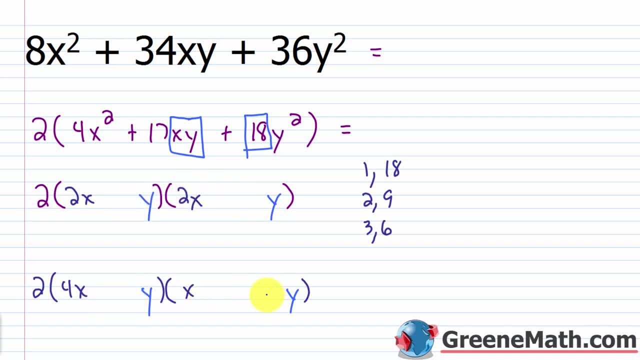 So it wouldn't work in this one. It might work in this one, but I'd have to try this configuration here: an 18 here and a one here, So just think about four times 18, that would give us 72.. 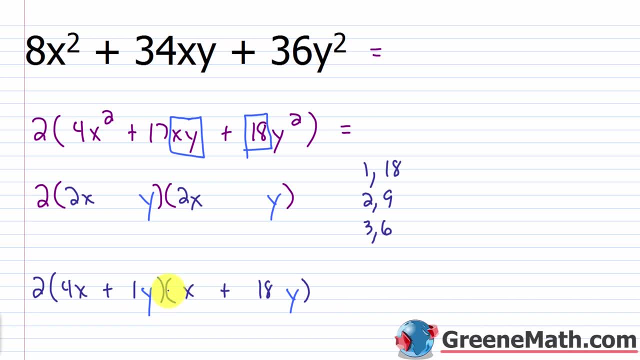 And you'd have one times one, which would be one. So 72 plus one would be 73. So that's not gonna work out in either one. So you can go ahead and get rid of that. All right, Let's erase this. 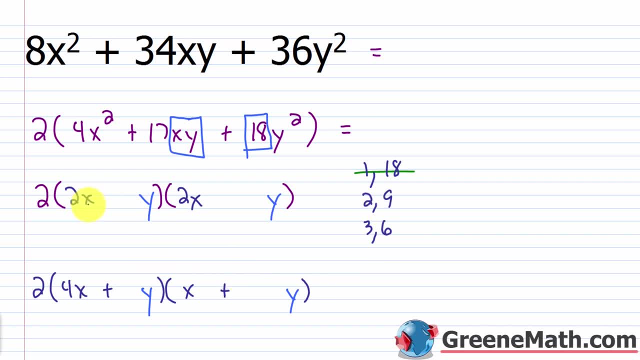 Next, let's think about two and nine. So in the first one I can't use it at all, Again because I'd have to put a two somewhere. I can't use a two here or here because I'd have a common factor of two. 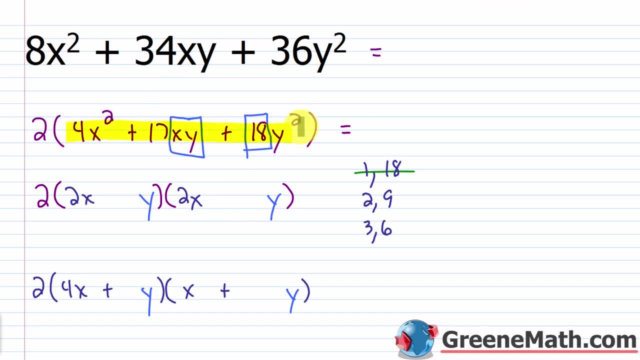 There's no common factor in this right here that we're trying to factor. I know there's one up here, but again, we've already pulled that out, So there shouldn't be one in any of the binomials there, So it's not gonna work there. 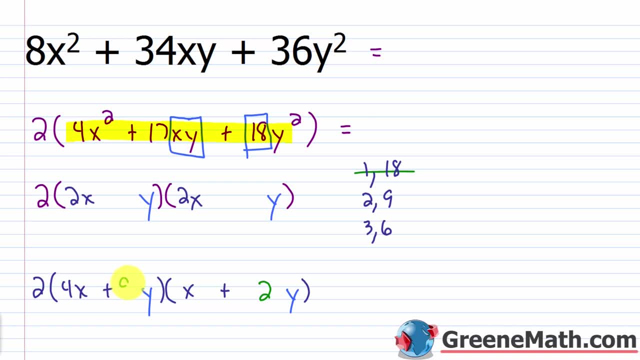 In this one. I can put a two here and put a nine here. I can check that scenario. So four times two would be eight. Nine times one would be nine. Eight plus nine is 17.. So we have found what we need. 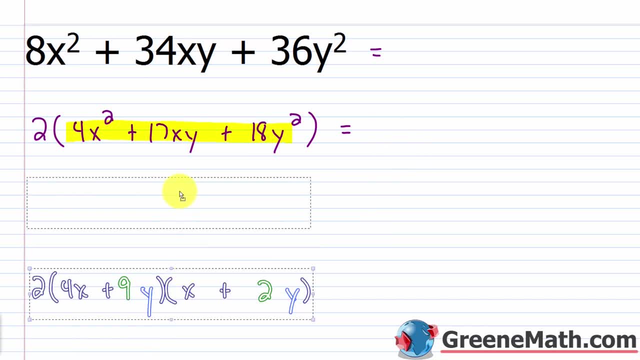 So let's erase everything. Let me just kind of slide this up so we can check it through FOIL. So I'm gonna put my two out in front: Four x times x is four x squared. My outer four x times two y would be positive eight x y. 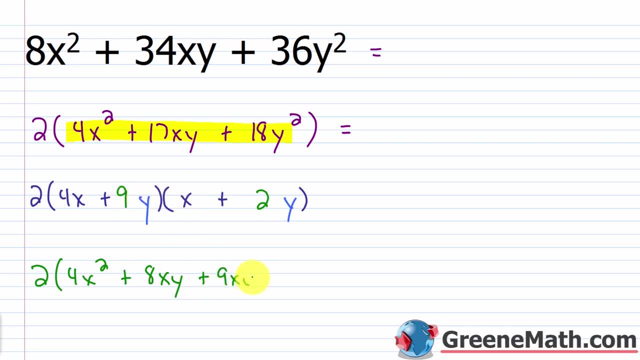 My inside nine y times x would be positive nine x. And my last nine y times two y would be positive 18 y. squared Again, when we think about those two middle terms here, eight x y plus nine x y would be 17 x y. 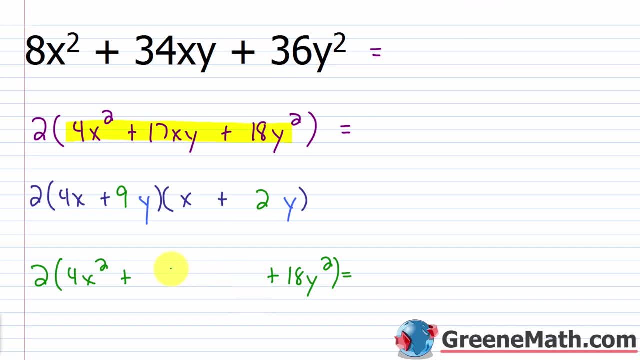 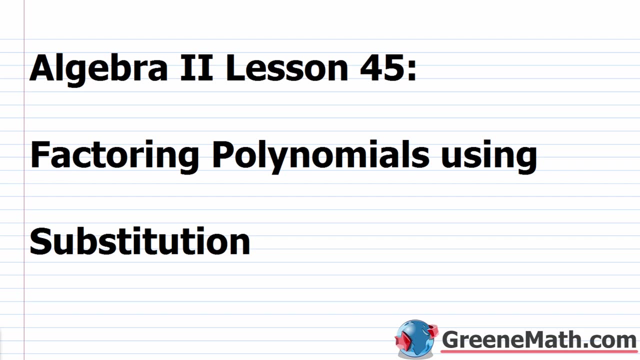 So let's just erase this and put plus 17 x y, And if I distributed that two I'd be back to eight x squared plus 34 x y, plus 36 y squared. Hello and welcome to Algebra 2, Lesson 45.. 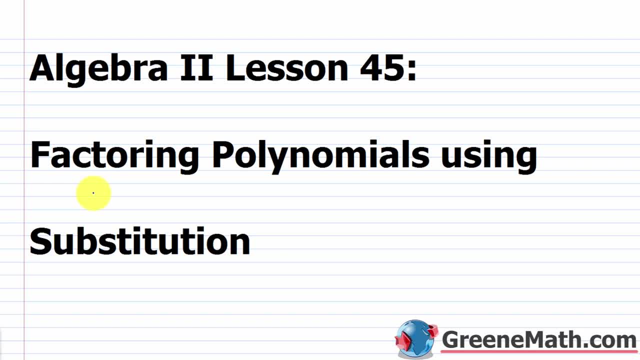 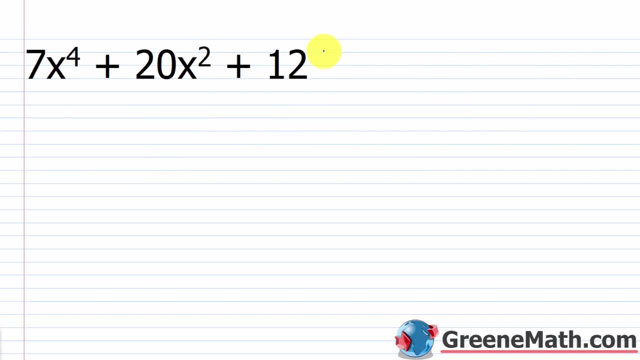 In this video we're gonna learn about factoring polynomials using substitution. So in some cases we can factor a more complex polynomial by making a substitution. So I wanna jump right in and just look at an example here. So let's suppose you see seven x to the fourth power. 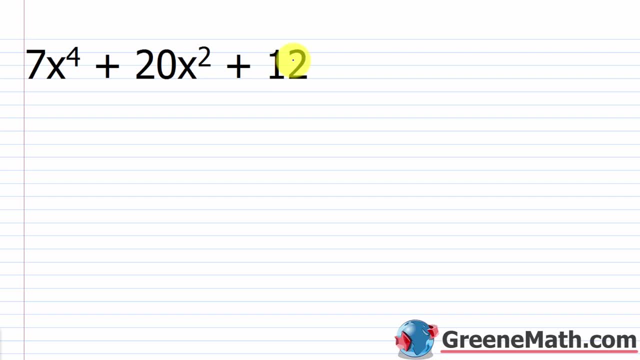 plus 20 x squared plus 12, and you're asked to factor this. Well, you might look back at me and say, well, I don't know how to do that. I'm used to seeing something that looks like this: A x squared. 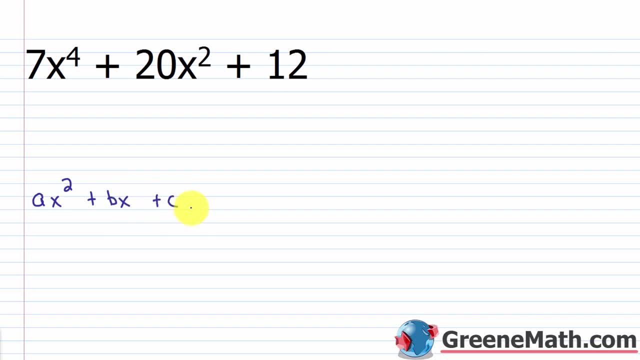 A squared plus bx plus c. Now I've got something times x to the fourth power plus something times x squared plus some constant. So the way this works, if you look at this particular problem, I could rewrite this and I just have to show this to you. 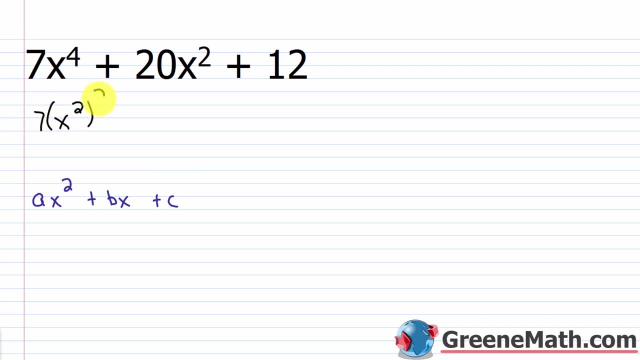 as seven x squared, that's squared. Now if I take x squared and I square it, what do I have? I have x to the fourth power. So I haven't changed anything, I just rewrote it. Then, plus 20 x squared. 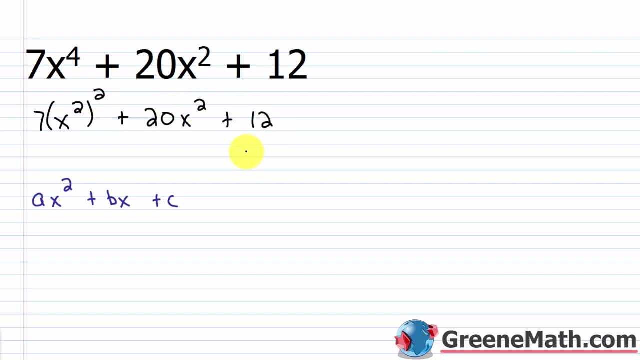 Then plus 12.. Now the benefit or the reason to writing it like this. you see that I have an x squared here and an x squared here. So what if I made a substitution and I let a variable be equal to or the same as my x squared? 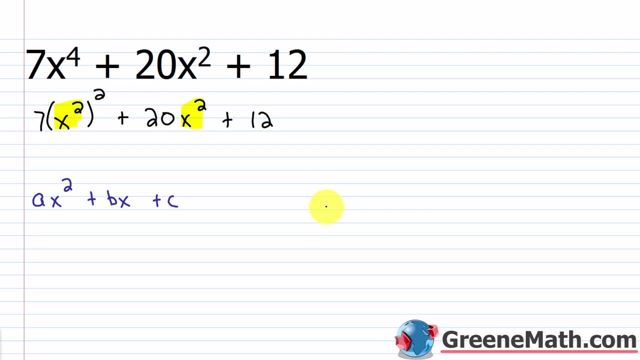 So that variable could be whatever you want. You could use y or z or q or n or whatever you want to do. Let's just go ahead and use u, So u is going to be equal to x squared. So that means everywhere I see an x squared. 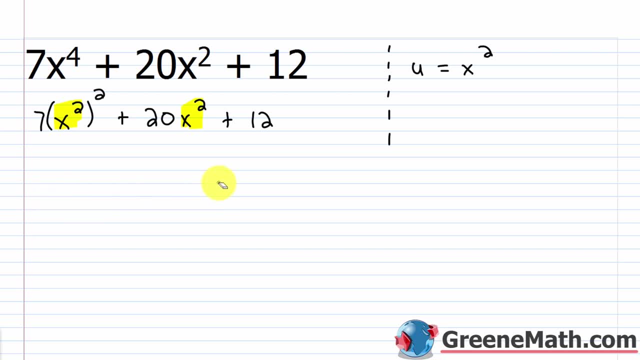 I'm going to plug in a u. Let me erase this. We don't need this anymore, And so I'm going to rewrite this problem as seven. I have an x squared there, So I'm going to write a u, Then that's squared. 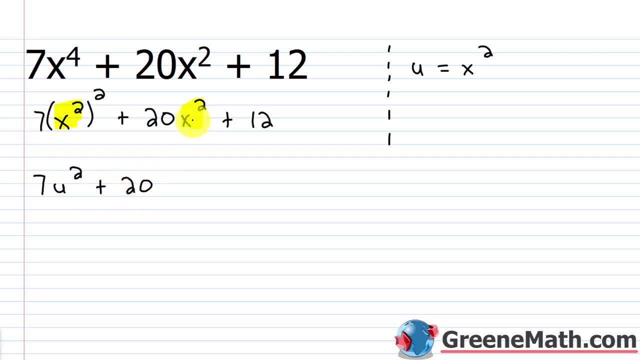 So seven u squared plus, we'd have 20.. Then I have an x squared, So that's going to be a u, Then plus I have 12.. So now, if I look at this right here, it matches a format that I'm familiar with. 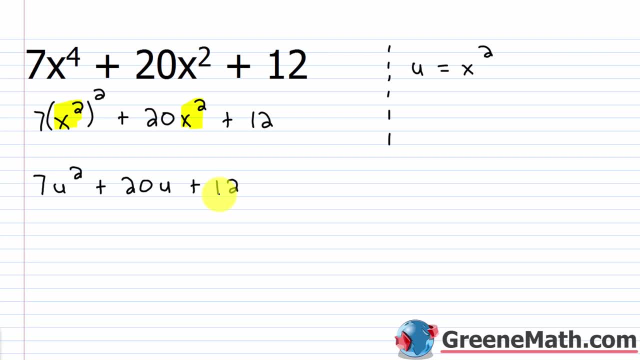 Okay, Very easy to factor this. We just talked about it. We can use reverse FOIL if we want, or we can also use a method that relies on factoring by grouping. I prefer to use factoring by grouping, So let's go ahead and factor this guy. 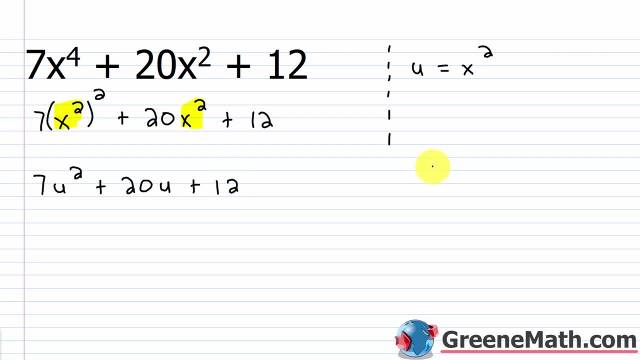 I would want two integers whose product is seven times 12. That's 84.. So the product is going to be 84. And then the sum is what The sum is to that middle coefficient, So a sum of 20.. So think about factors of 84.. 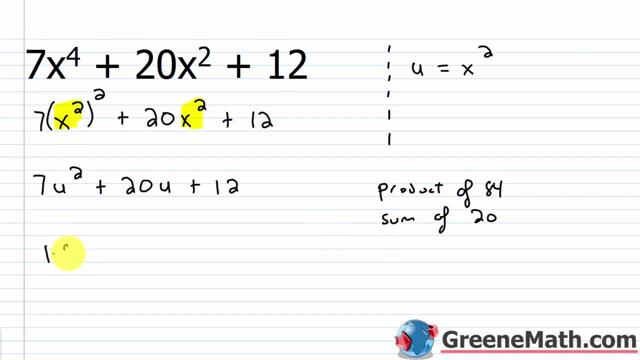 You think about 84. It's what You got, one times 84. That's obviously not going to work right, Because the two integers have to sum to 20. Then you've got two and 42. That wouldn't work. 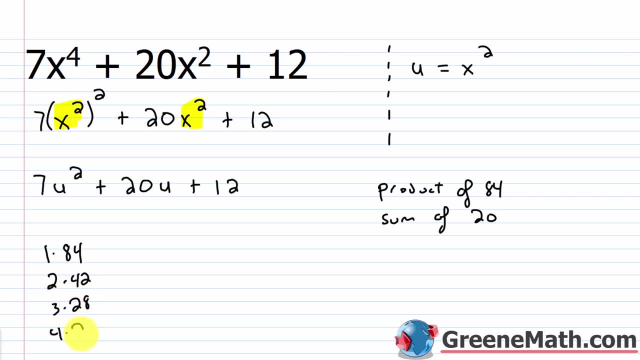 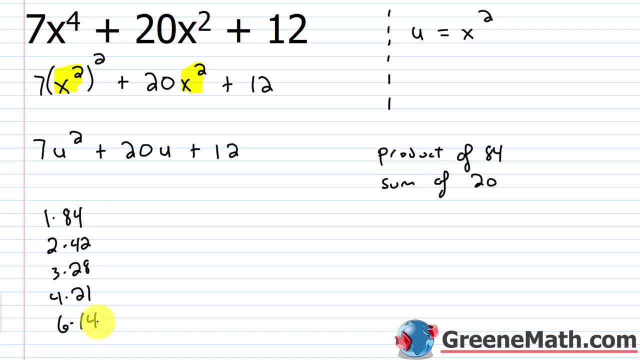 You've got three times 28,, which wouldn't work, Four times 21,, which wouldn't work. It's not divisible by five, but it is divisible by six. It's six times 14.. Now You've got 14 sum to 20.. 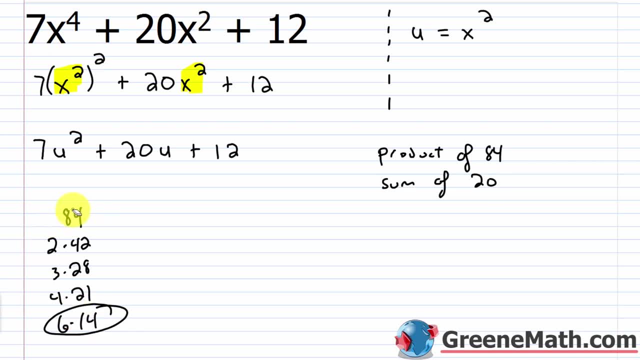 So that's your magical combination there. So let's erase this. We know what we need to erase this. So we take those two integers and we rewrite the middle term. So I would say that I have seven u squared plus I'll put 14 u, plus I'll put six u and. 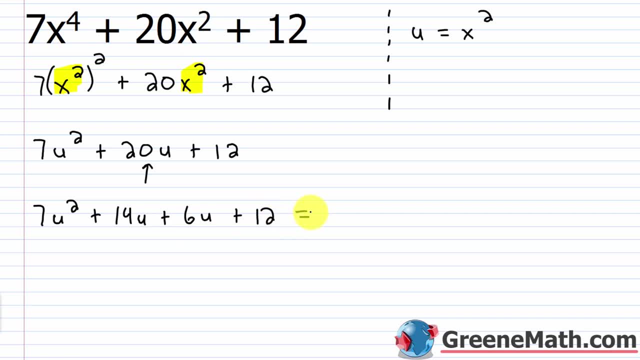 then plus 12.. Now I'm going to factor using grouping, So I'm going to take the GCF out of each Group. So from the first two I'm going to pull out a seven u and that's going to leave me with. 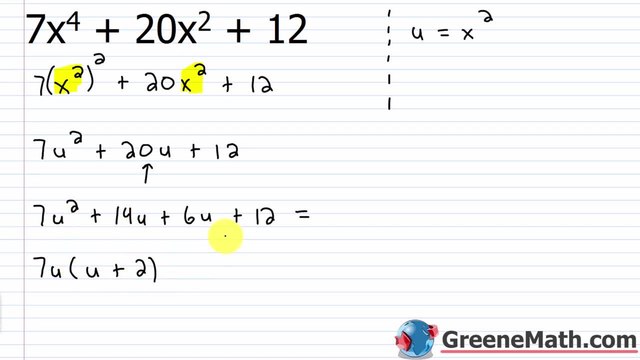 what? I'd have a u plus a two from the second group, I'm going to pull out a six and I'm going to have a u plus a two, So I can pull out the common binomial factor of u plus two And that's going to give me one. that's going to give me u plus two, that quantity times. 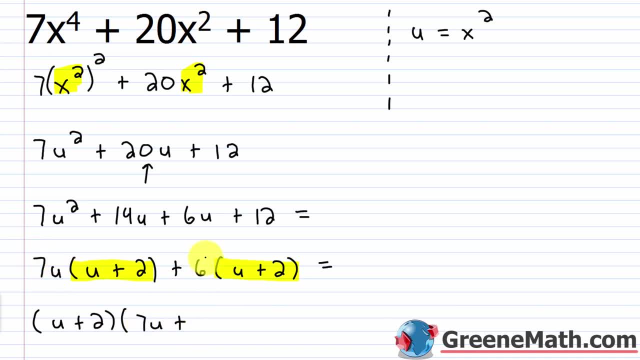 what's left. I'd have seven You there, So u plus two. that quantity times the quantity seven, u plus six. So if I'm taking a test or I'm doing my homework and I'm asked to factor this, can I report? 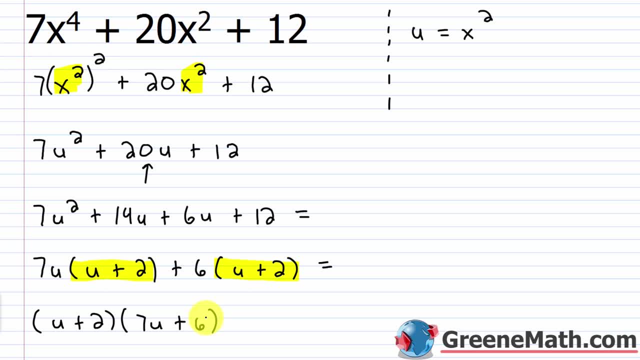 this as my answer. No, I made a substitution to make it easy on myself, So I've got to substitute back in the end. If u is equal to x squared, that means I can take every u that I have, Okay, So there's a u here and here and I can replace it with x squared. 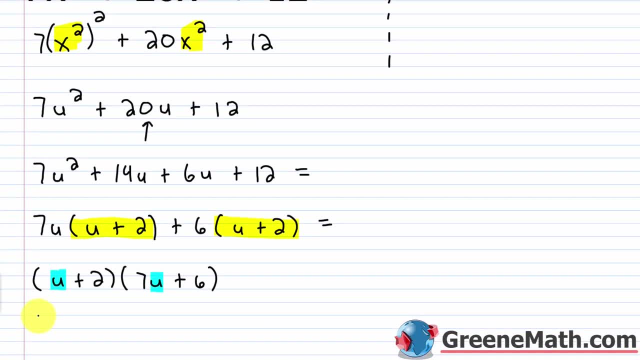 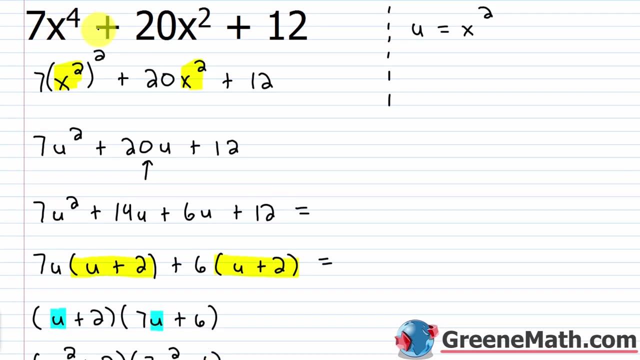 Okay, So let's say that my answer is what It's x squared plus two, that quantity times the quantity seven. Again you've got a u there, So x squared plus six. So I have factored this seven x to the fourth power plus 20, x squared plus 12 as the quantity. 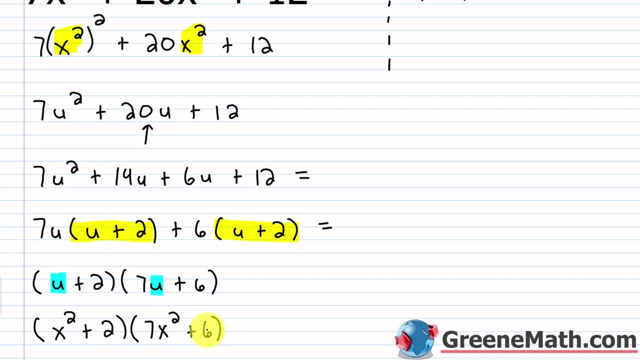 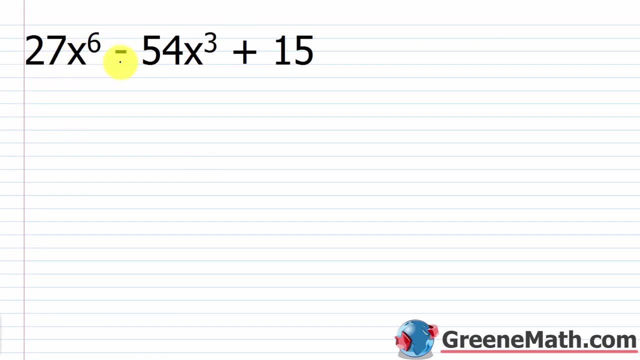 x squared plus two times the quantity seven x squared plus six. Again just using a simple substitution, Let's take a look at another example. So we have 27 x to the sixth power minus 54 x cubed plus 15.. So before we do anything, we should notice that everything here is divisible by three. 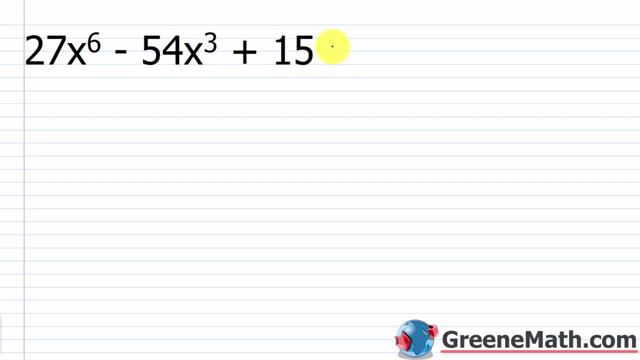 So I want to make sure I pull that out so I don't forget about it or have additional factoring in the end. So if I pulled out a three to start this, 27 would now be a nine and still have my x to the sixth power, then minus 54 divided by three would be 18, then x cubed, then plus. 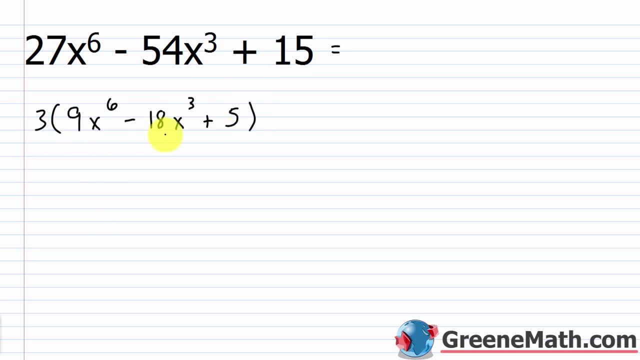 we know 15 divided by three, So I want to do this one more time. So if I pull out a three to start this, 27 is a nine and still have my x to the fifth power. So I'm going to do this one more time. 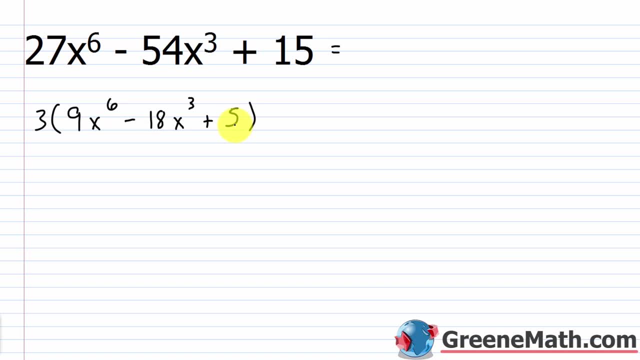 We're going to do this one more time, I'm going to do this one more time. So I'm going to do this one more time. So I just want to factor this one more time. I'm just going to do this one more time and you can see it's five. 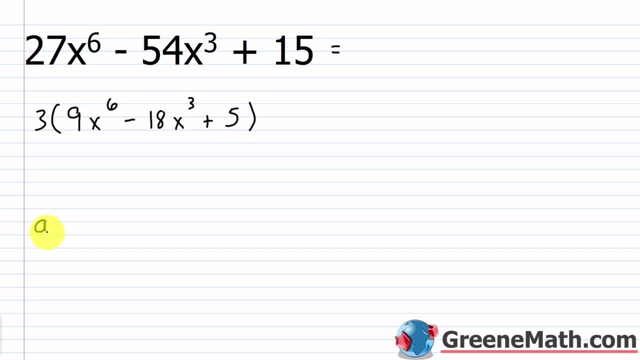 So this is what I'm working on now. I just want to factor what's inside the parentheses. Now, again, we can use a substitution. If you look at what we normally try to factor, it's ax squared plus bx plus c. You think about this exponent as a one, this exponent as a two. 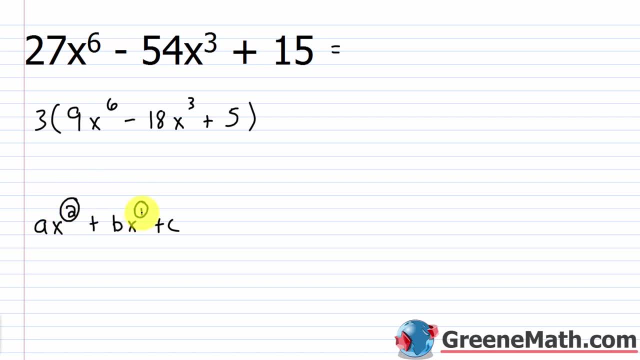 So this exponent here is double this exponent here. In the last example we looked at we had an exponent that was a 4, which was double the exponent of a 2.. In this example here you have an exponent of a 6 that's double the exponent of a 3.. 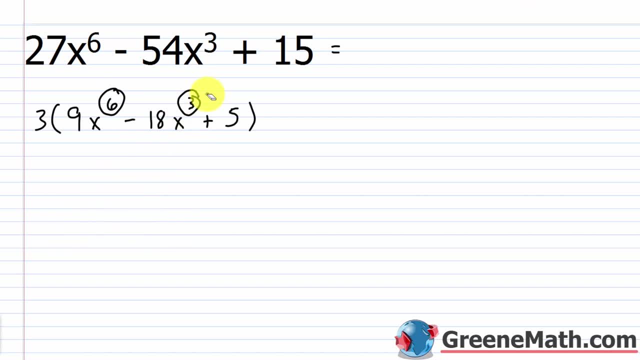 So when this occurs, you can use a substitution And you're going to take a variable. let's say u or q or n or whatever you want to do. Let's just say z for this example. Let's say z, That's going to be equal to the variable raised to the smaller power. 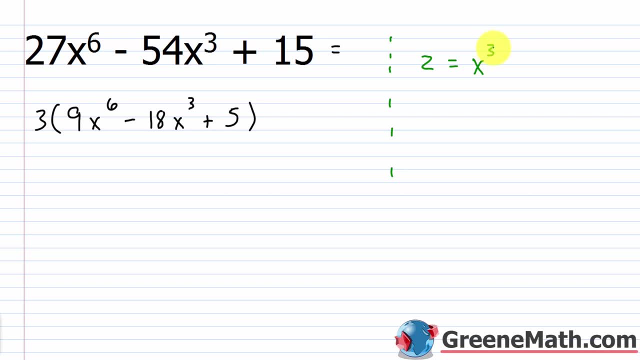 So z is equal to x cubed in this case. Now, since this exponent is double this one, what I can do using my rules of exponents, I can rewrite this. I'll put 3 times- it's out of parentheses- 9x cubed. 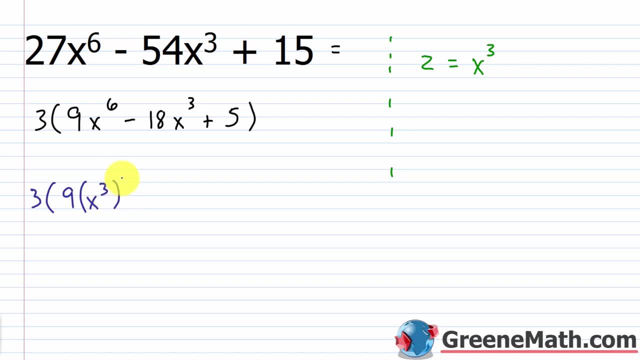 So you want to match that. But I'm doubling this exponent, so I'm just going to raise it to the second power or square By the rules of exponents. x cubed squared would be x to the sixth power. Then you'd have minus 18x cubed, then plus 5.. 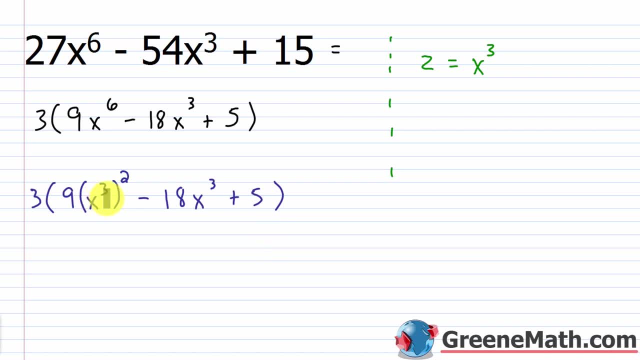 And the reason you write this this way is so it's obvious what you're going to do when you substitute Here's x cubed and here's x cubed. So what I'm going to end up doing when I make my substitution: I'm going to say that I have 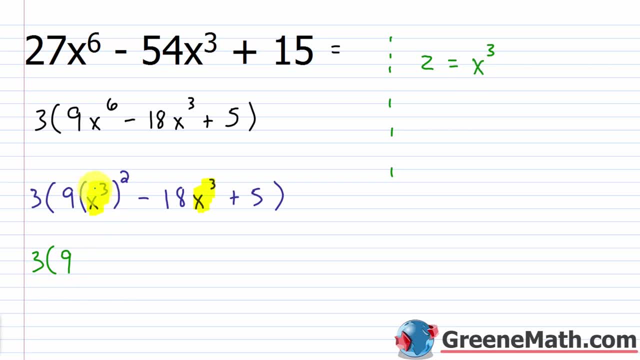 3 times inside of parentheses 9.. This right here will be replaced with a z. z equals x cubed. I have x cubed. I have x cubed right there. so that would be z and then squared. 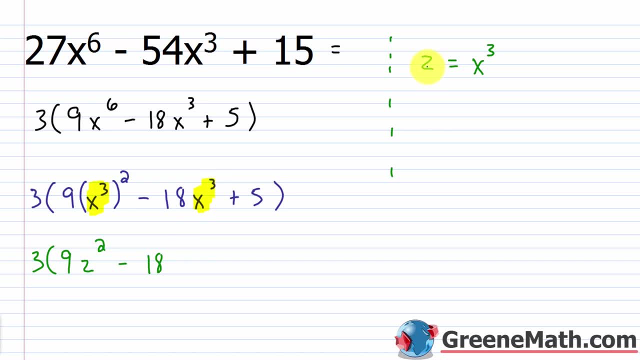 Then minus. I have 18 times. Here comes x cubed again. so I'm going to substitute with a z and then plus 5.. So all I have to do now is just factor this, as I normally would. Once I'm done, I go back and I resubstitute, and I have my answer. 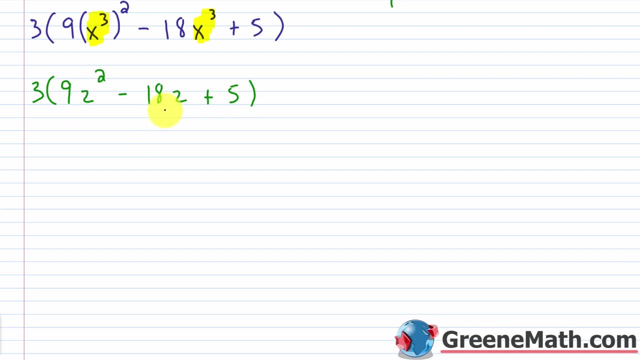 So give me two integers whose sum is negative 18.. So the sum is negative 18.. And whose product? okay, Whose product is 9 times 5, or 45. Now we know from the rules of signs that this has to be a negative and another negative. 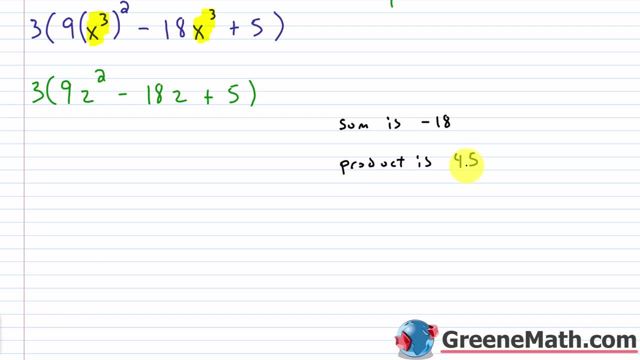 Negative plus negative is negative. Negative times negative is positive. So I'm thinking about negative values. But in thinking about that, I can just think about positives and then just switch over. So think about the factors of 45. You've got 1 and 45,, which obviously wouldn't work. 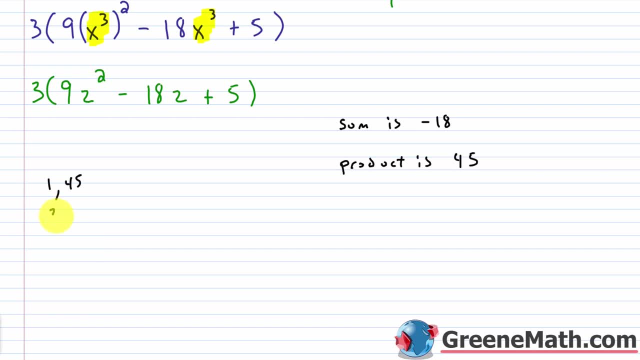 It's not even so. it's not divisible by 2.. It's 3 and 15,. 3 times 15 would be 45.. Now what's interesting here is: 3 plus 15 is 18,, but I just want negatives involved. 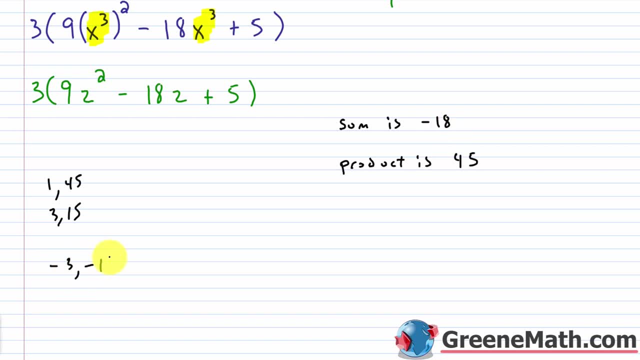 So I would think about negative 3 and negative 15.. That's what I want. Negative 3 times negative 15 is positive 45. Negative 3 plus negative 15 is negative 18.. So I'm going to use those two integers to rewrite my middle term. 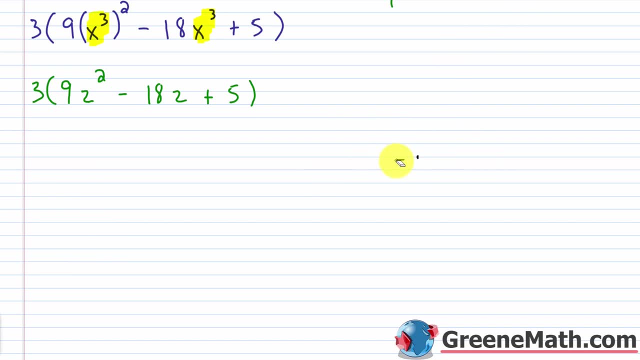 Okay, So let me erase this, And I'm going to say that this is equal to: we're going to have 3 times- it's out of parentheses- 9z squared minus 15z minus 3z plus 5.. 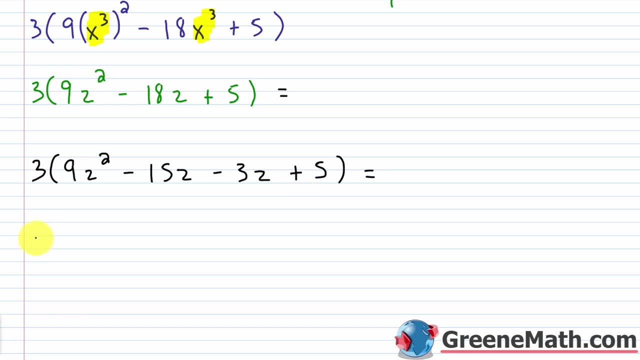 And so I'm going to use factoring by grouping in the middle. here I'm going to have my 3 out in front From the first group, the first 2, I could pull out a 3z, So pull out a 3z. 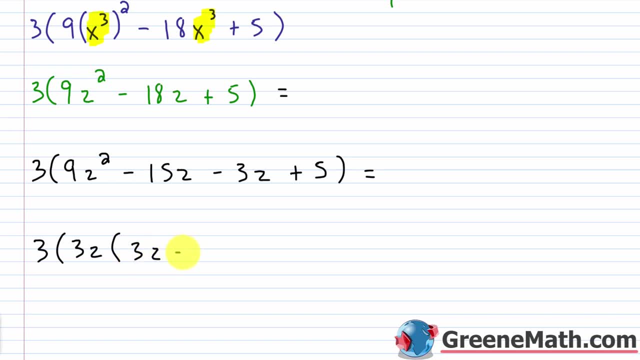 That would leave me with A 3z minus a 5.. Then in the second group I have negative 3z and I have 5.. Well, if I look at trying to get a common binomial factor, I just want opposite signs. 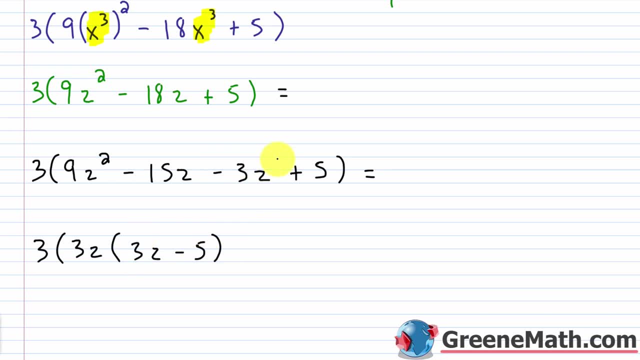 I want positive, 3z and negative 5.. So just pull out a negative 1., Pull out a negative 1. You can change the signs. This would be 3z, This would be negative, 5.. And so now I have that common binomial factor that I'm looking for. 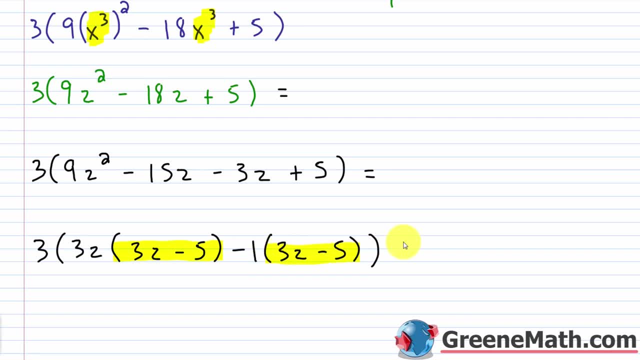 This 3z minus 5.. Okay, So I can take that and factor it out. I'd have a 3 out in front. Factor out the quantity 3z minus 5 and it would be multiplied by what's left. 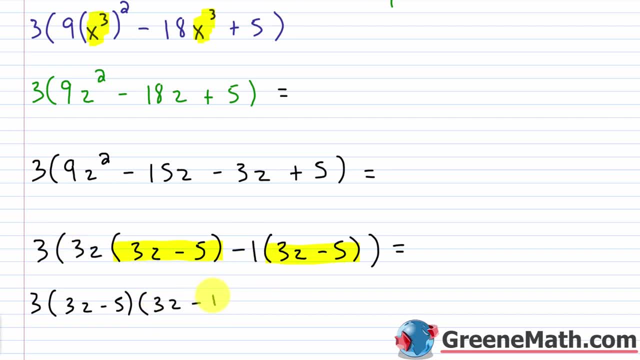 You'd have a 3z here minus a 1 here. So this factors into 3 times the quantity 3z minus 5 times the quantity 3z minus 1.. Now am I done with this problem? No, I substituted to get here. 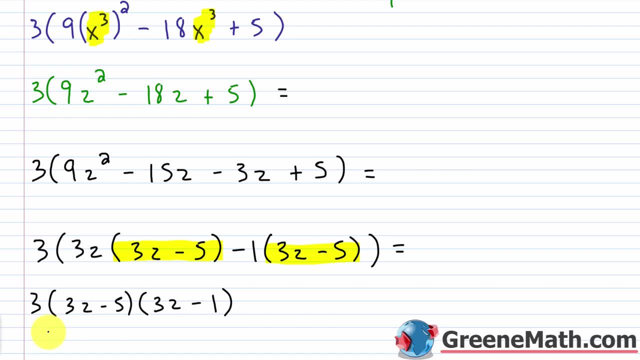 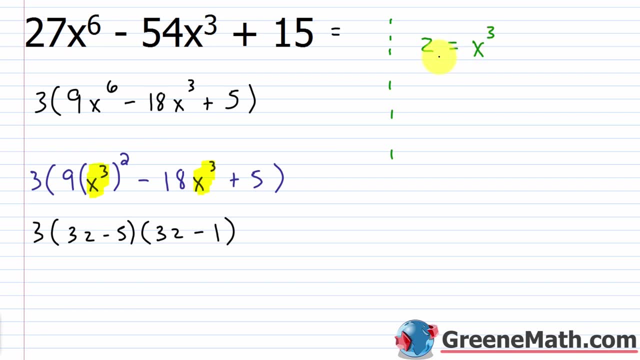 So I've got to substitute to finish this up. So let me erase this and I can kind of move things up. All right, So we know that we substituted a z for x cubed. So everywhere there's a z I can just go back and put x cubed. 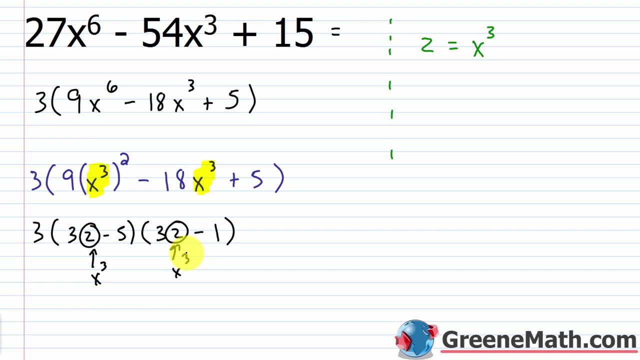 It's just that simple X cubed here and x cubed here, and I'm going to have my answer for the original problem. So it would be 3 times the quantity 3x cubed minus. 5 times the quantity 3x cubed minus. 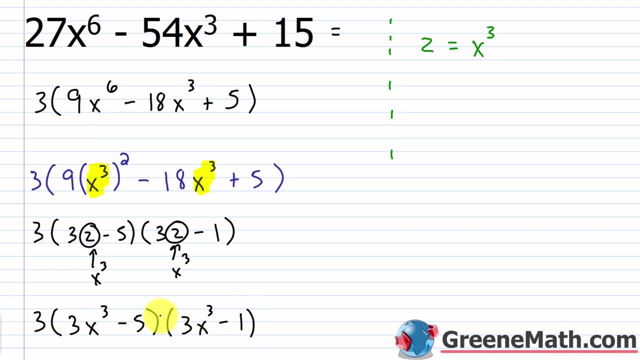 1. If you don't believe me, go ahead and FOIL this out. You'll get a result. Multiply that result by 3 and you'll get back to 27x, to the 6th power minus 54x cubed. 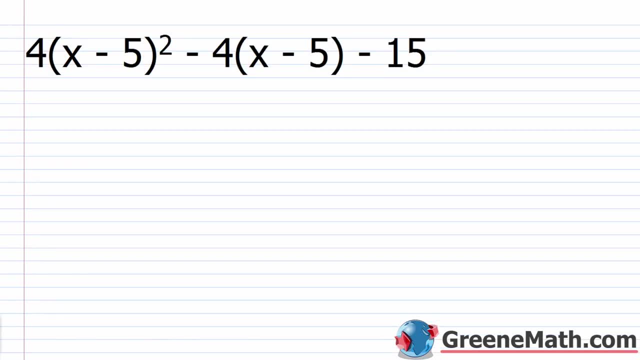 plus 15.. All right, So let's take a look at another one. So I just want to show you another scenario where you can use substitution. We have 4 times the quantity x minus 5 squared minus 4 times the quantity x minus 5 minus. 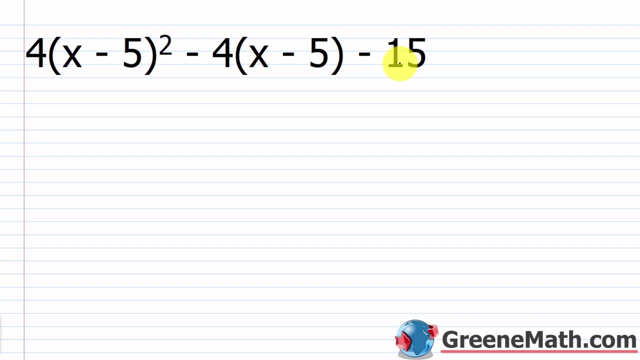 15.. So if someone said, go ahead and factor this again, you might have a little bewildered look on your face. But again, if you see something that's common, like the quantity x minus 5, I could just replace that with a variable. 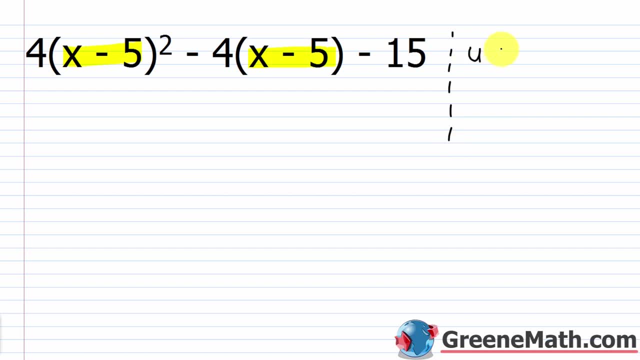 So I can say, hey, I can let u, or let's just go ahead and do q. I can let q be equal to the quantity x minus 5.. So everywhere I see an x minus 5, I could replace it with a q. 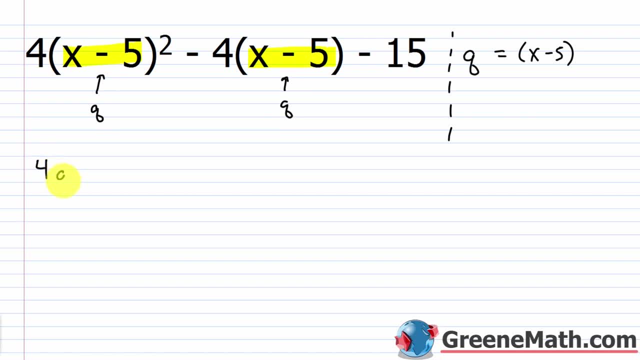 So what would that give me? Well, I'd say: 4q squared, That's 4.5.. That's 4.5. That's 4.5.. So that's 4.5 cubed minus 4q, minus 15.. 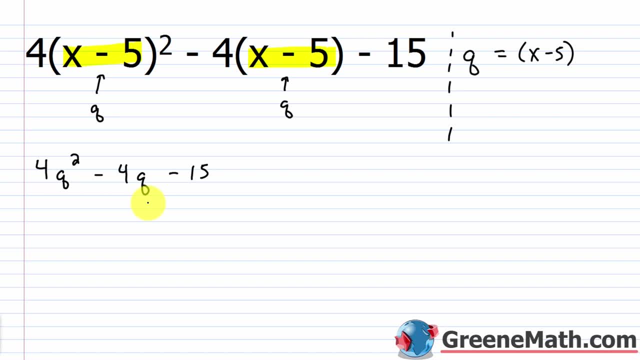 Can I factor this? Yes, I can. I can find two integers whose product is negative 60. So the product is negative 60 and whose sum is negative 4. So the sum is negative 4.. So we're going to have to think about this a little bit more, because we have a negative. 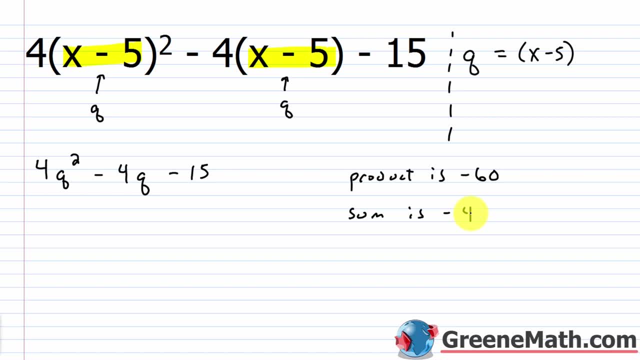 product. So that means we have one positive integer and one negative integer. so let's think about some combinations that we can do, so for factors of 60. i'm going to throw out things like 1 times 60 or 2 times 30. they're too far away. then next you'd have 3 times 20. 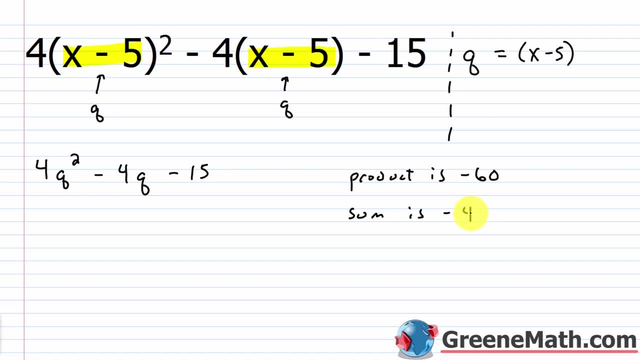 also too far away. you've got 4 times 15. that wouldn't work. you've got 5 and 12. that wouldn't work. then you come to 6 and 10. so if i had 10 minus 6, that would give me 4. but i want negative. 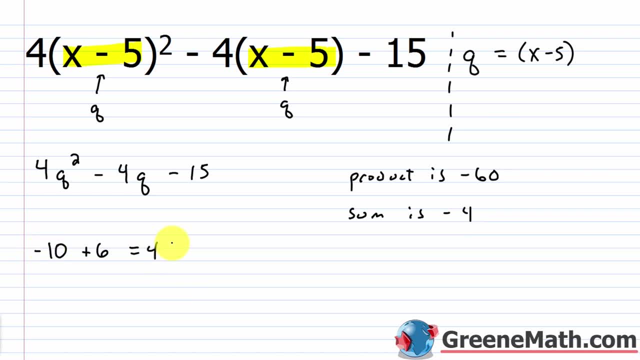 4. so i'd have to put positive 6 and negative 10 and that would give me a negative 4. so i'm looking for a negative 10 and a positive 6. negative 10 times 6 is also negative 60, so let's use these. 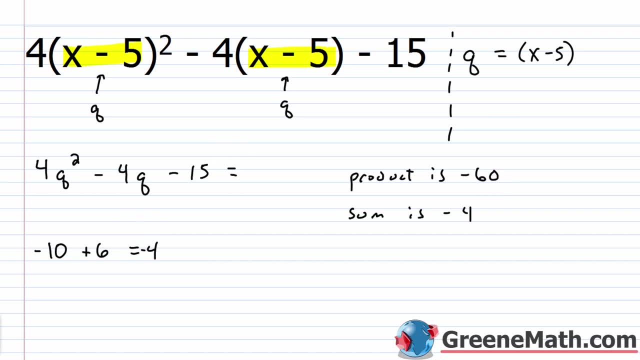 integers to rewrite that middle term. let's erase this and say that we have 4q squared minus 10q plus 6q minus 15. so if i use my factoring by grouping, i can pull out the numbers and i can see that i have 4q squared minus 10q plus 6q minus 15. 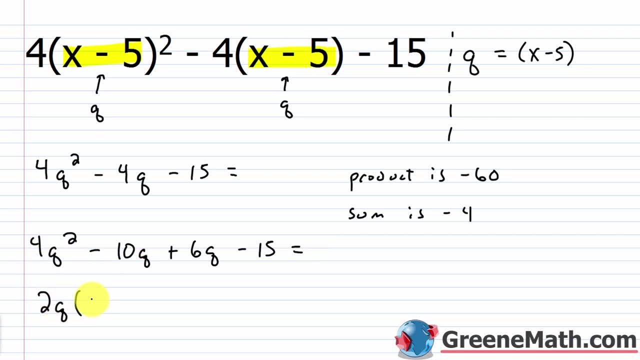 so i can pull out a 2q from the first group. that would leave me with 2q minus 5. from the second group i can pull out a 3, so plus 3 times you'd have 2q minus 5. so if i factor out the common, 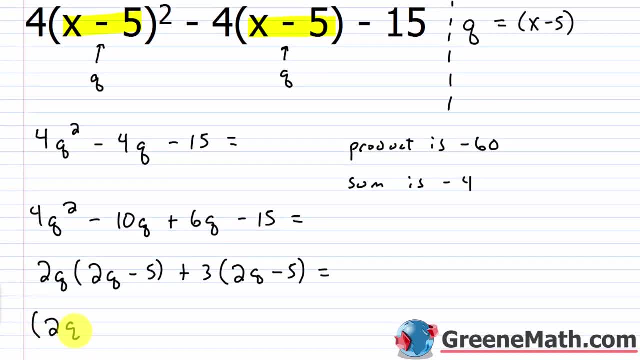 binomial factor, i'd have the common 2q minus 5 that's pulled out and then times what's left, which is 2q plus 3. so this is my factorization, but again i'm not done because q is representing x minus 5. so let me erase this up here and i'm going to substitute. 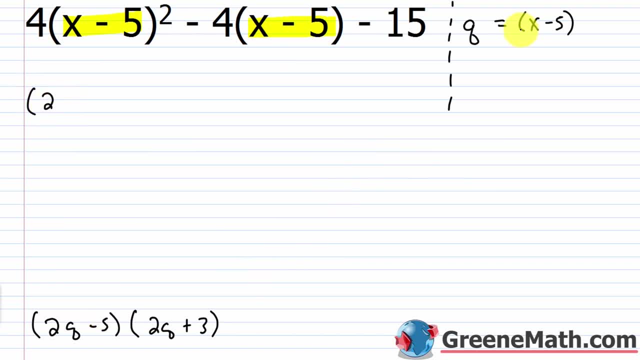 so inside of parentheses, i have 2. remember: q is the quantity x minus 5. make sure you use parentheses, they're very, very important, because 2 is multiplying this whole thing, then minus 5, then times, you have 2q, so 2 times the quantity x minus 5, and then plus 3. all right, so let's erase. 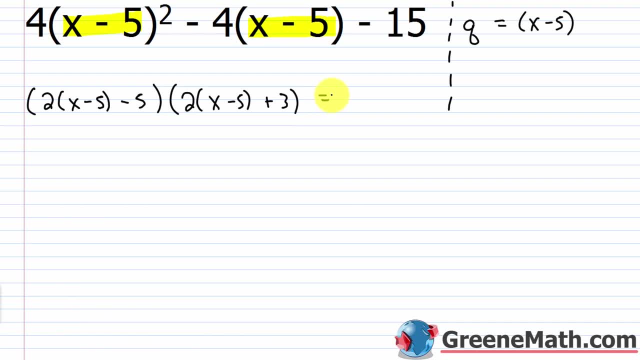 this and we would think about this. so if i go through and kind of simplify: 2 times x is 2x, 2 times negative 5 is minus 10, and then minus 5. well, negative 10 minus 5 is negative 15. so let's. 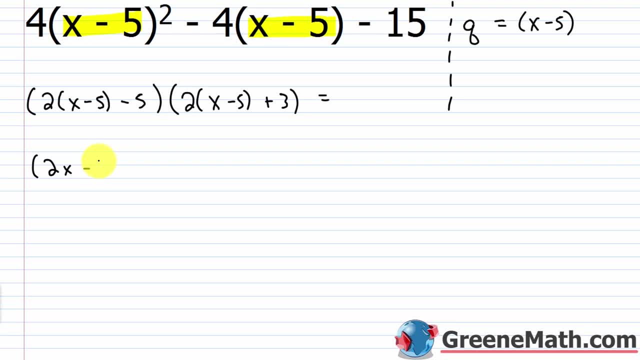 write 2x minus 15 and then for this one, 2 times x is 2x, and then 2 times negative 5 is negative 10, and then you have plus 3, negative 10. plus 3 is negative 7. so i have factored this into 2x minus 15. that quantity times the quantity 2x minus 7. now you 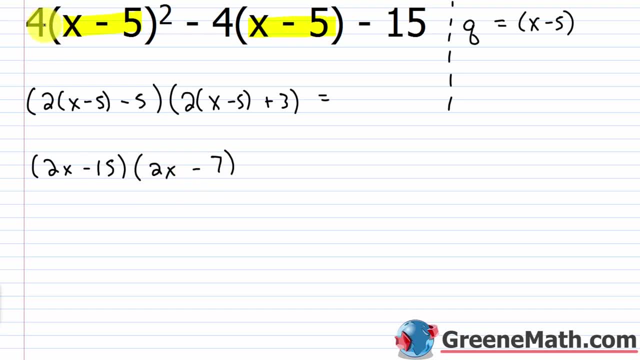 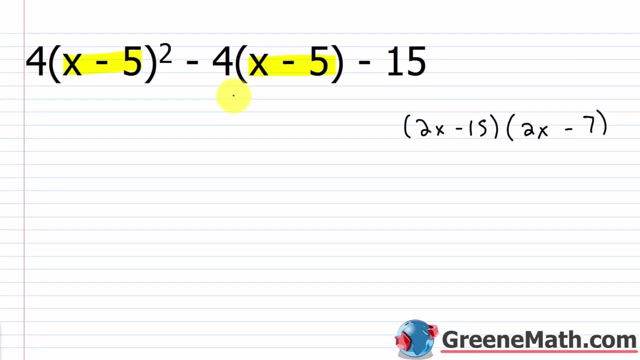 might sit there and say there's no way that this is the factorization of this, but in fact it is and i'm just going to put this off to the side and i'm going to prove that to you. and let's say you were to look at this problem and say, okay, i can't start out by just using distributive property. 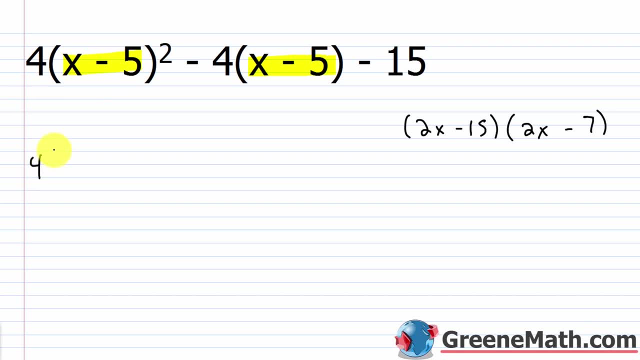 i've got to expand this, so i would have four times. we know how to do this from our special property, so i'm going to do this. this would be x squared minus 2 times x times 5. 2 times 5 is 10, so 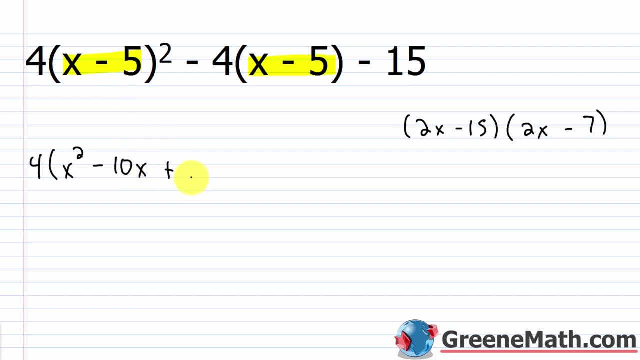 we'd have 10x and then plus this guy squared 5, squared is 25. so let me just stop and do the 4 times this. this would be 4x squared minus 40x plus 100. okay, so let me just erase this now for. 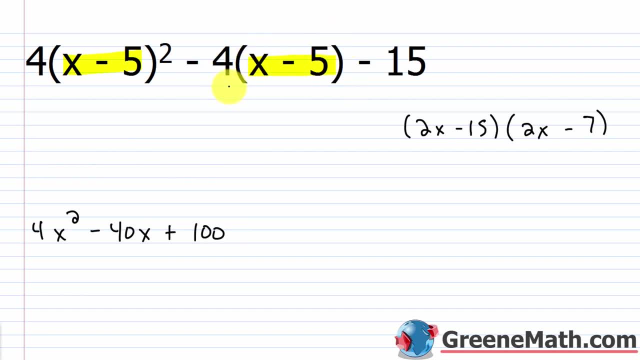 this one. i have a negative 4 times this. it's not squared or anything, so i can just use my distributive property. negative 4 times x minus 4 is negative. 4 times x minus 4 is negative. 4 times x is negative 4x. and then negative 4 times 5 is plus 20, and then you have minus 15.. okay, so we have 4x. 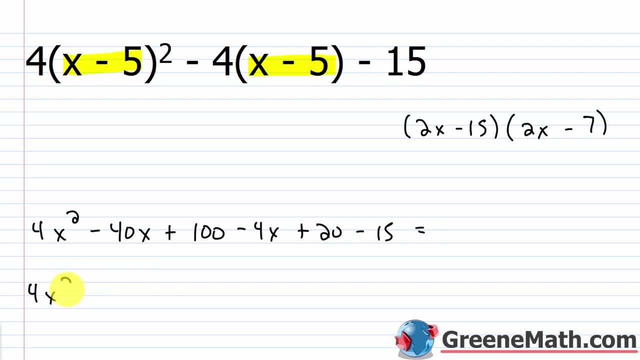 squared. nothing to combine with that. i've got negative 40x minus 4x, that's minus 44x. and then i've got 100 plus 20, which is 120 minus 15, which is positive 105.. now let me erase this and you 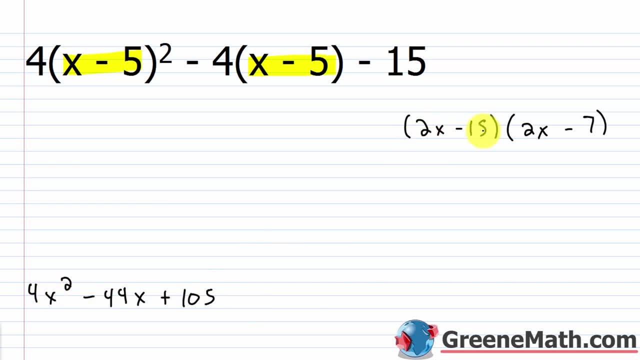 could do one of two things now: you could factor this into this or you could foil this into this. let's go ahead and foil this into this because it's a little bit quicker. so 2x times 2x would be 4x squared, the outer 2x times negative. 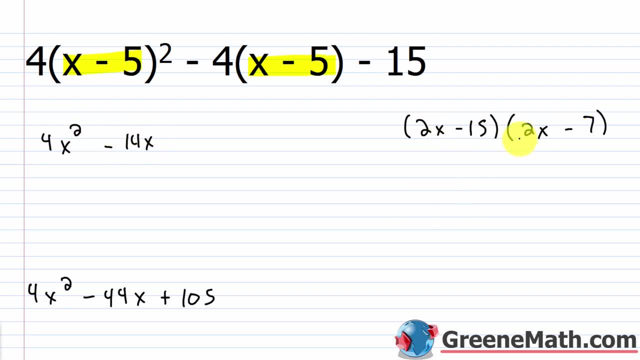 7 would be negative 14x. the inner negative 15 times 2x would be negative 30x and then the last negative 15 times negative 7 is positive 105. so if you combine like terms in the middle here, you see that you would get 4x squared. 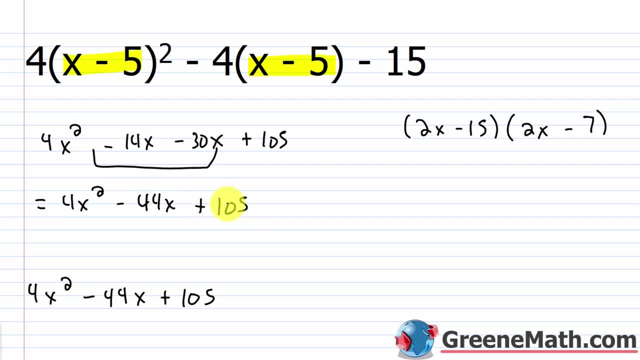 minus 44x plus 105, which is exactly what you have right there. so just a much quicker way to factor. think about having a factor. this versus what we factored, it was quicker in the end. right, just to make the substitution and then go back. hello and welcome to algebra 2, lesson 46. in this video we're 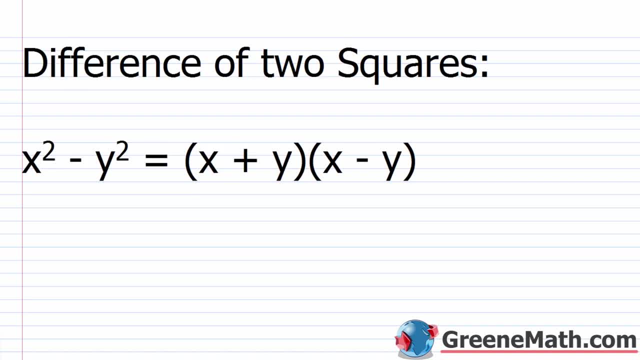 going to learn about special factoring, so we did a lesson on this back in algebra 1. but again, i think it's very important to review this because you're going to come up with a lot of questions. you're going to come across factoring scenarios that occur so frequently that it's super beneficial. 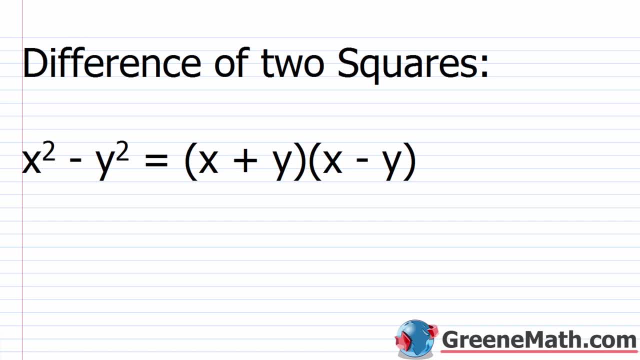 for you to memorize the generic formulas, and this can be used on your homework, your tests or something important like the sat or the act's, where they're timed and you have a certain amount of things and you just have to be as fast as you can. so i'm going to start out by talking about the 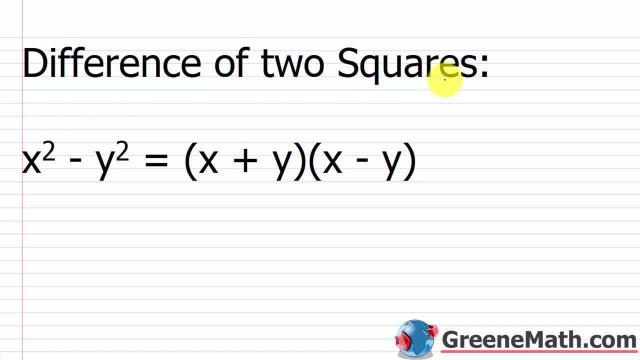 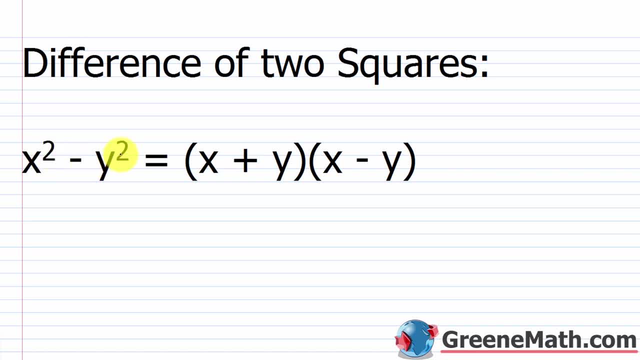 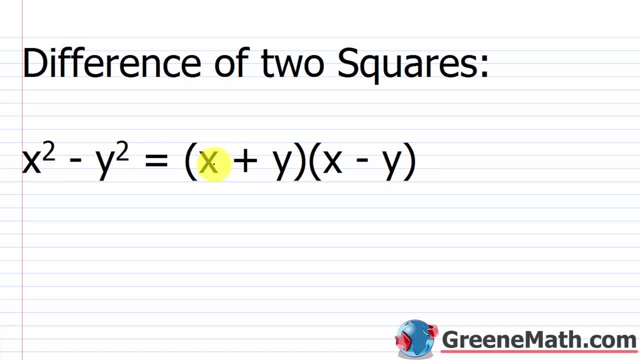 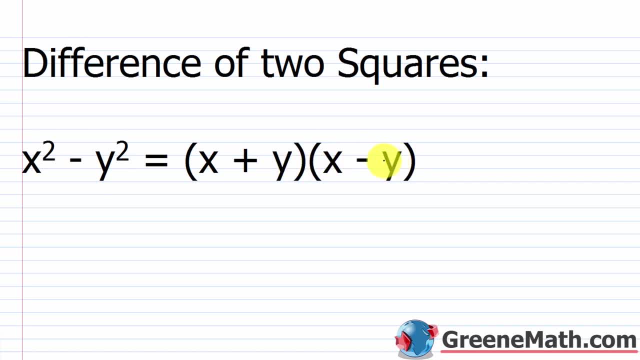 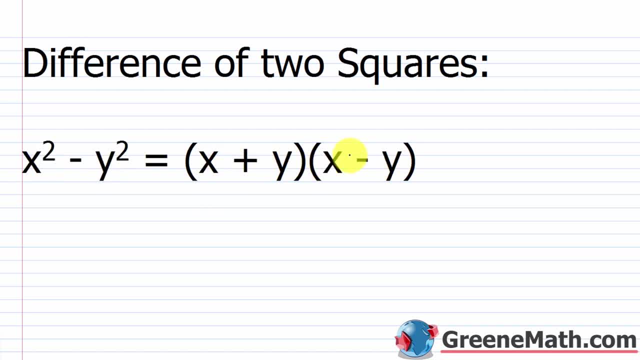 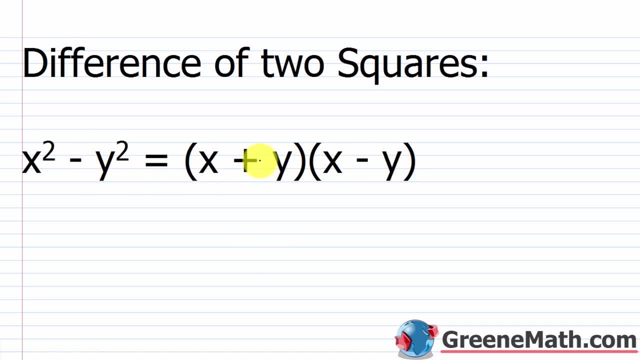 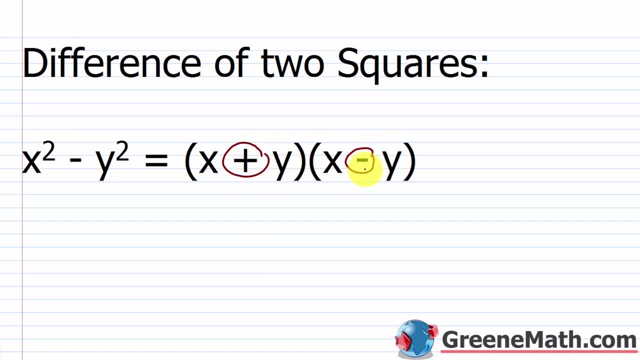 minus here. Now you could change that around and put the minus here and the plus here- wouldn't affect the answer. And this is based on the fact that if I do FOIL- let's say I have the quantity x plus y times the quantity x minus y- what's going to happen is those two middle terms are going. 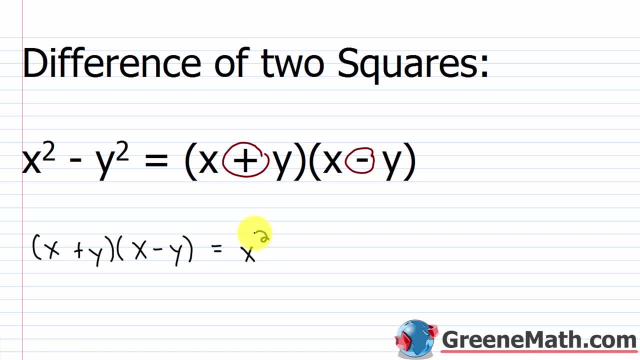 to cancel each other. X times x is x squared, the outer x times negative y is minus xy, the inner y times x is plus xy and the last y times negative y is minus y squared. So you can see that this is going to cancel and you're left with x squared minus y squared. 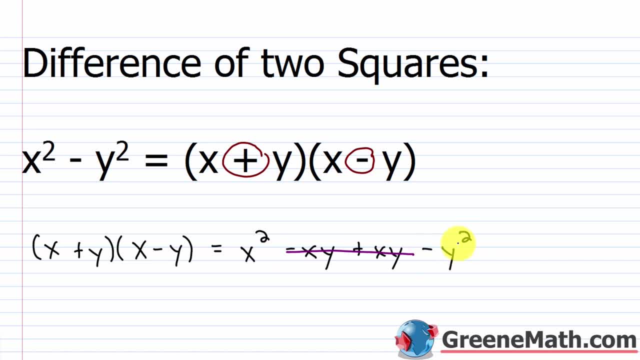 So if I see something squared minus something else squared, I can quickly factor it using this technique. So let's just say I saw something like I don't know, x squared minus 4.. We know x squared is a perfect square, but is 4?? 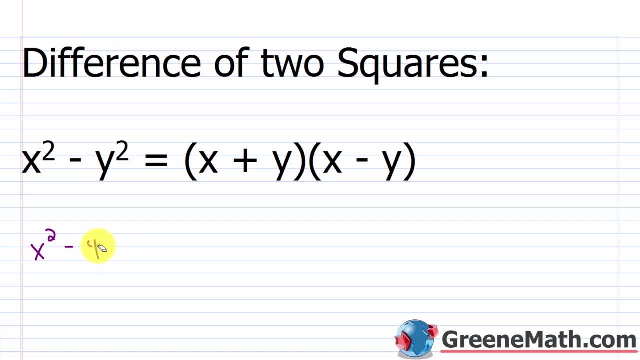 Well, of course, 4 is 2 squared, So make this simple on yourself and just rewrite this as 2 squared. Let's say this is 2 squared. So then, following this format, we just set up the parentheses. I know one of these is plus and one of these is minus. 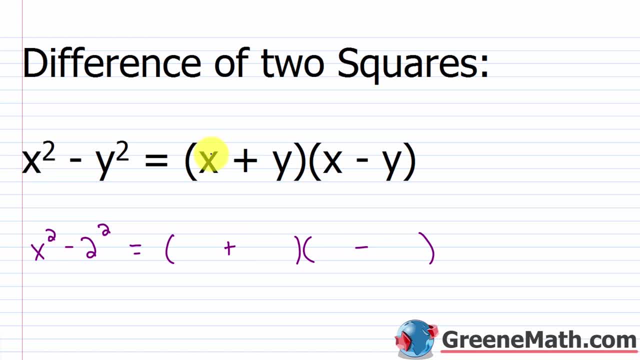 The first thing that's squared- in this case that's x- appears again in the first position of each. So whatever squared is going to appear in the first position of each, And then the second thing that's squared- in this case it's y. 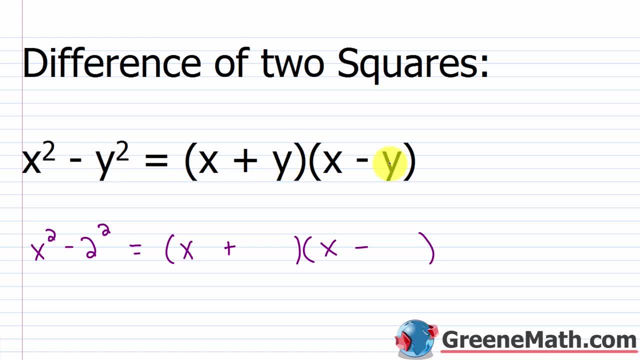 It's going to appear in the second position of each. So we've got a y there and a y there. Here what's squared is 2.. So that would appear here and here And again from your special products formulas. you know that the quantity x plus 2 times 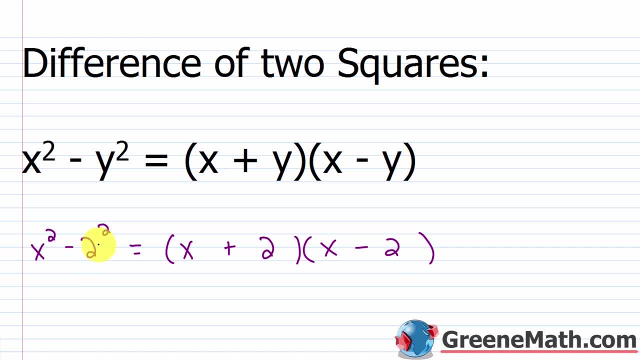 the quantity x minus 2 would be x squared minus 2 squared or x squared minus 4.. Okay, you can go back and forth between the two. So let's say I gave you something like 4x squared minus 1 and I told you to factor it. 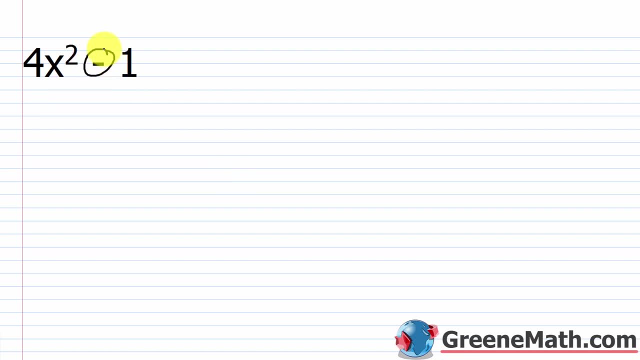 Well, the first thing is there's two terms only. Okay, There's a minus sign, So I'm immediately thinking the difference of two squares. So what I'm going to ask myself is: is this a perfect square? Yeah, I could write this as 2x that quantity squared. 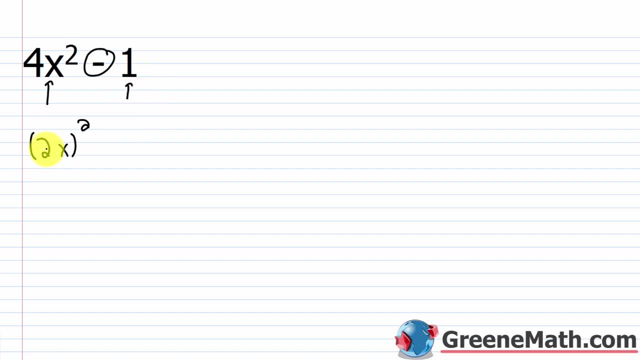 And then is this a perfect square? Yeah, 1 squared is 1.. So I could write 2x, that quantity squared minus 1 squared. So if I transform this into this, I can use my little formula: Set up your parentheses. 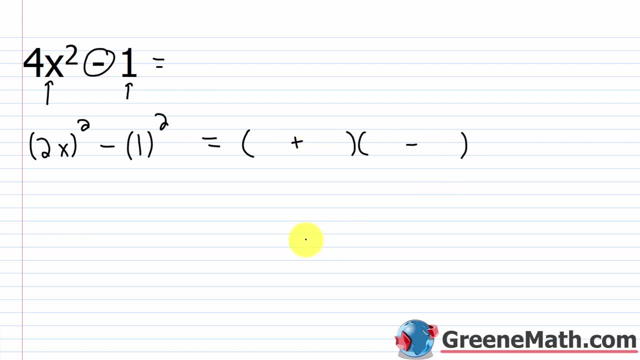 This is how I remember it: Put your plus and your minus. Whatever is squared first goes in the first position of each. 2x is what's squared, So put a 2x here and a 2x here. Whatever is squared second goes in the second position of each. 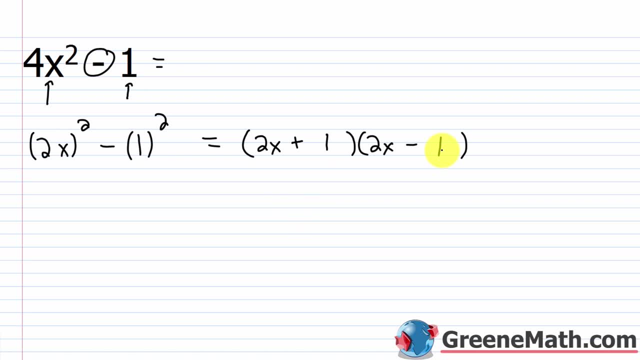 And that's it. I've got the quantity 2x plus 1 times the quantity 2x minus 1.. If you want to use FOIL and check it, 2x times 2x is 4x squared. The outer 2x times negative 1 and the inner 1 times 2x would cancel. 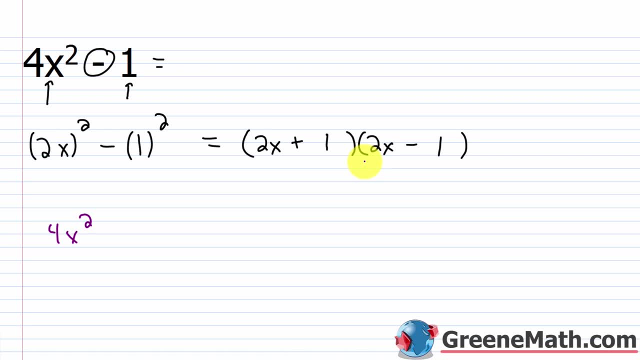 You'd have positive 2x and negative 2x. that's gone. The last is 1 times negative 1, which is negative 1 or minus 1.. So you have 4x squared minus 1 and you start out with 4x squared minus 1.. 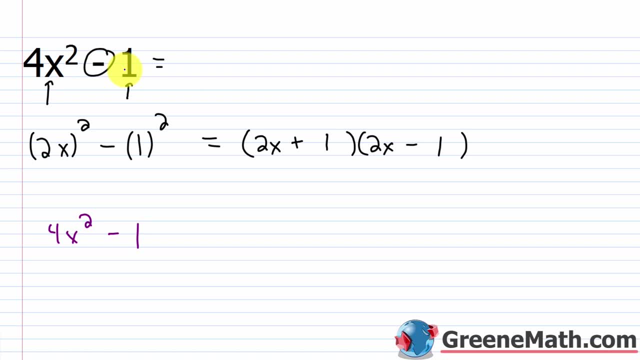 So again, a very, very simple and fast approach to factor this. All right, let's take a look at another one. So we have 25p squared minus 16. So again, two terms only and a minus sign. So immediately you should be thinking about the difference of two squares. 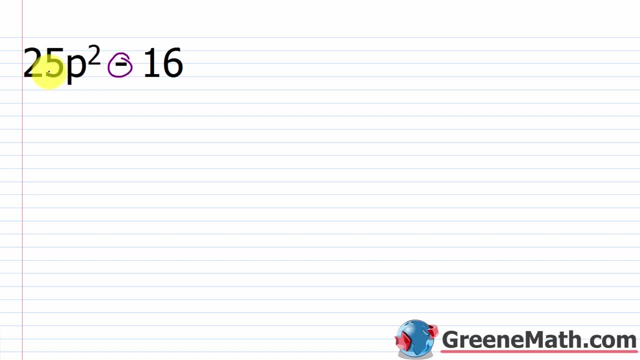 So is 25 a positive 2x and negative 2x? Is 25 a perfect square? Yeah, it's 5 times 5 or 5 squared. We know p squared is a perfect square, So I could write this as 5p- in parentheses- squared. 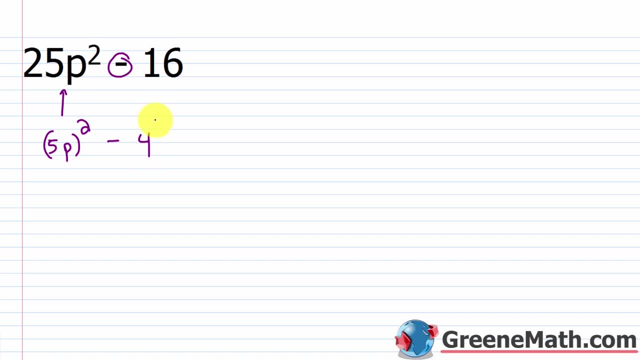 Then minus is 16, a perfect square. Yes, it's 4 squared. So what I can do is I can factor this Again, set up your parentheses, put a plus and a minus and then whatever squared in the first position- in this case that's 5p- is going to go here. 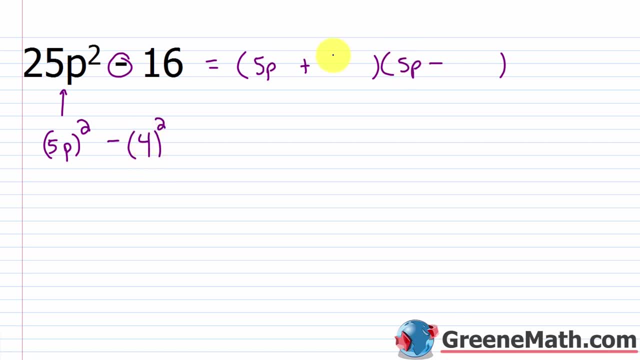 And here Whatever squared in the second position is going to go here and here. First position goes in the first position of each, Second position goes in the second position of each and we get our answer. This factors into the quantity 5p plus 4 times the quantity 5p minus 4.. 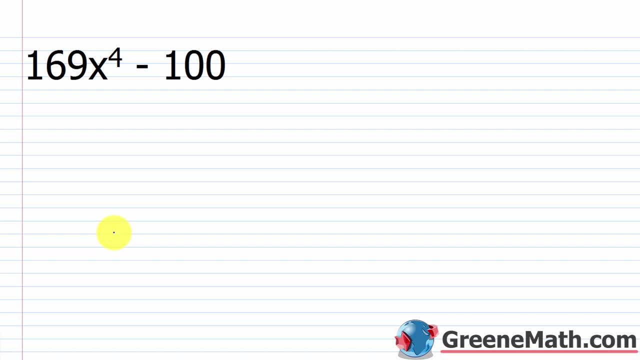 All right, for the next one, we're looking at 169x to the fourth power minus 100.. So again, two terms and you got a minus sign. So we're looking for the difference of two squares, So 169x to the fourth power minus 100.. 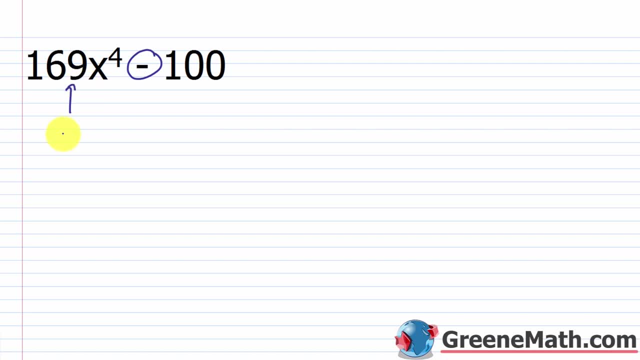 So again, two terms and you got a minus sign. So 169 is what It's, 13 squared. So let me write 13 there And x to the fourth power is what I can really think about this again using the rules of exponents, as x squared squared. 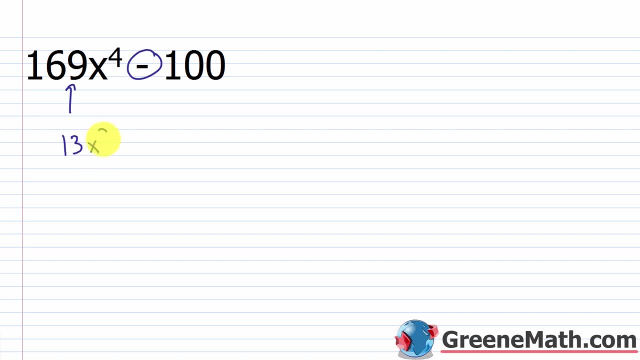 Okay, So what I want to write is 13x squared. and then this thing right here, inside of parentheses: the 13x squared would be squared. This, mathematically, is the same as this, and I just rewrote it. 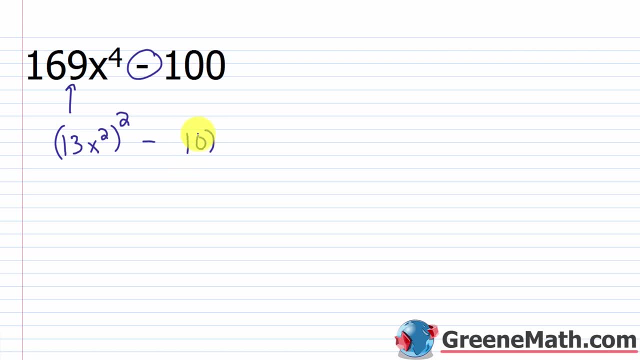 Then minus. We know 100 is 10 squared. Let's write 10, and that's squared. So to factor this again, set up your parentheses very, very easy: One is plus, one is minus. Let me put minus and then plus. 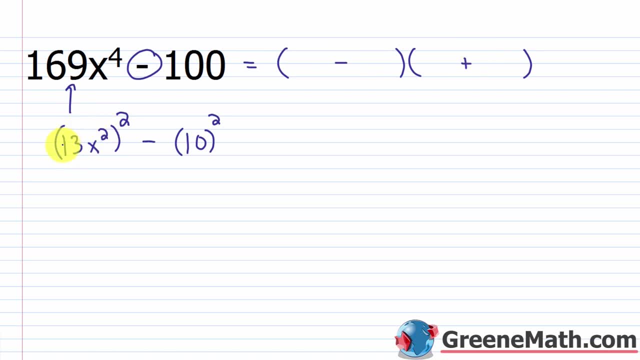 The order doesn't matter- And then whatever is squared in the first position- here it's 13x squared- is going to go first in each case. so 13x squared and then 13x squared, And then whatever is squared in the second position- in this case that's 10,- is going. 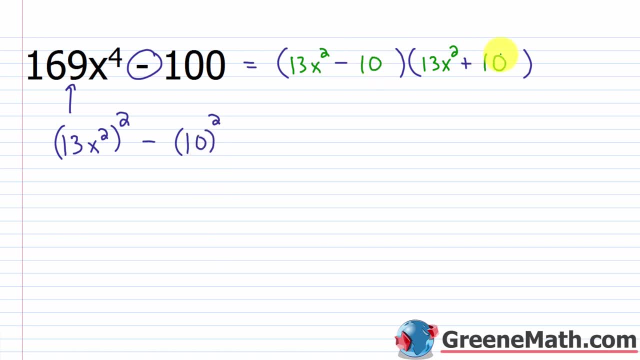 to go in the second position of each. So a 10 here and a 10 here. So we've factored this as the quantity 13x squared minus 10 times the quantity 13x squared plus 10.. All right, So let's look at the next one, which is where we talk about perfect square trinomials. 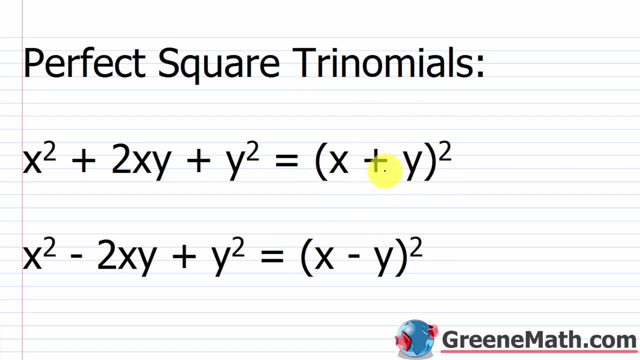 So we all know from special products that the quantity x plus y squared turns into x squared plus 2xy plus y squared. So obviously we can factor and go from x squared plus 2xy plus y squared to the quantity x plus y squared. 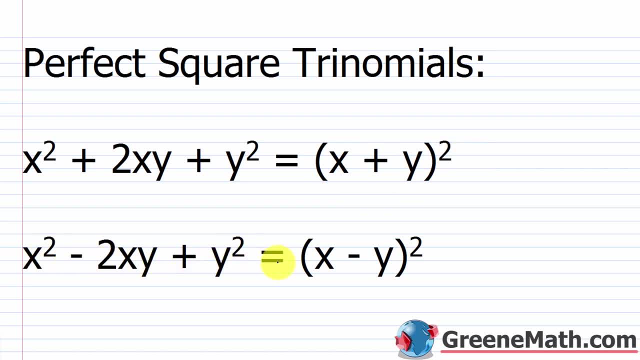 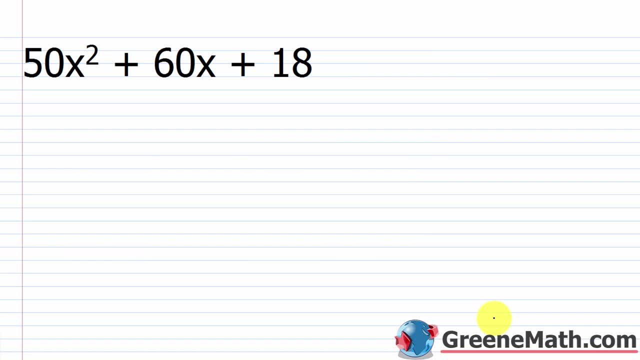 Now if I have x squared minus 2xy plus y squared, I can factor that into x minus y, that quantity squared. Let's take a look at an example of this. We have 50x squared plus 60x plus 18.. 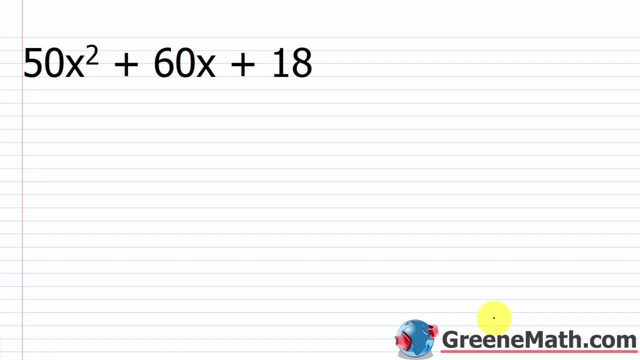 So let's say, I tell you to factor this Now: when you look at 50, you would say: well, that's not a perfect square. When you look at 18, you'd say: well, that's not a perfect square. 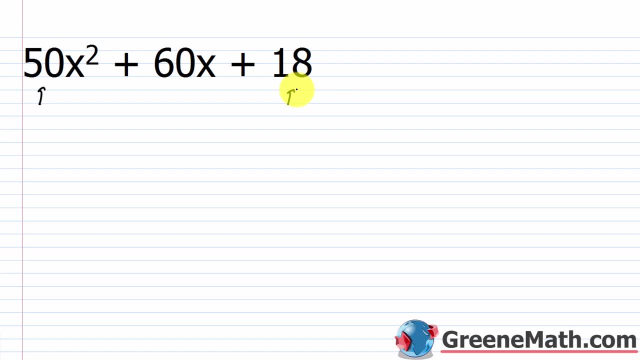 So you might give up on this idea of it being a perfect square trinomial. But before you do that, just realize that everything here is divisible by 10.. So you might give up on this idea of it being a perfect square trinomial. But before you do that, just realize that everything here is divisible by 10.. So you might give up on this idea of it being a perfect square trinomial, But before you do that, just realize that everything here is divisible by 10.. 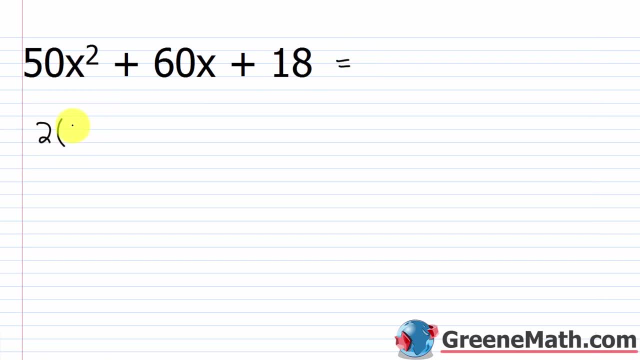 So you might give up on this idea of it being a perfect square trinomial. But before you do that, just realize that everything here is divisible by 10.. So if I start out by just pulling a 2, out inside the parentheses, that I have 25x squared. 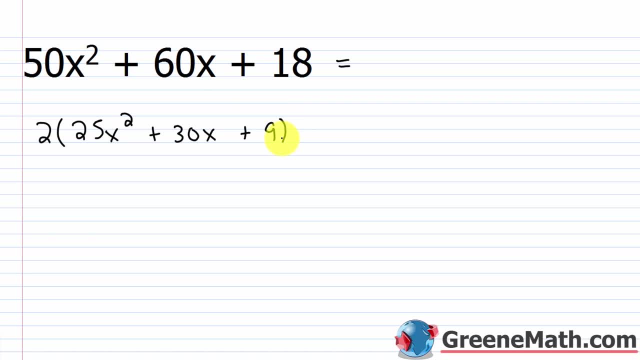 plus 30x plus 9.. So now, if I think about what's going on, I know 25 is a perfect square And I want to check this. 25 is a perfect square. It's 5 squared, X squared is a perfect square. 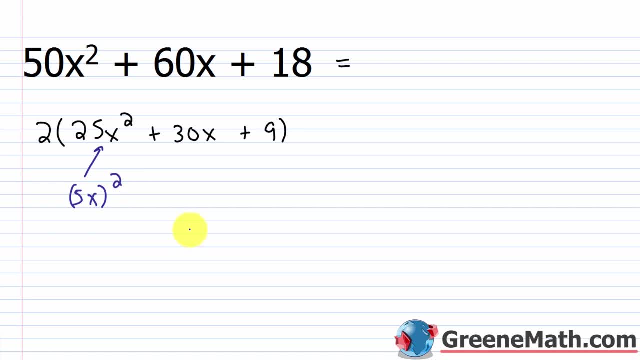 So I could write this as 5x, that amount squared Now. Now, But wait a minute- Is 9 a perfect square? Well, yeah, 9 is 3 squared. Okay, Now what we check is this middle term 2 times this times. this. 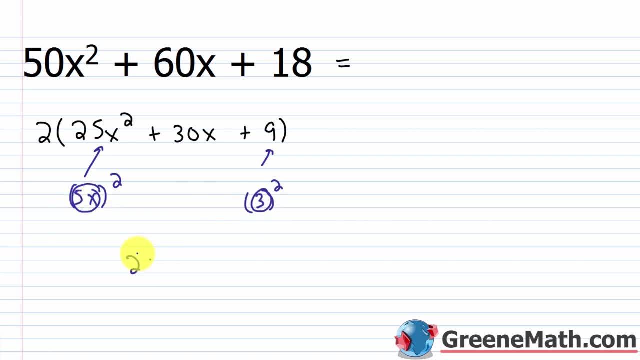 2 times 3 is 6.. 6 times 5 is 30. Times x is 30x. So 2 times 5x times 3 does equal 30x. So it all checks out. So that means I can factor this into what. 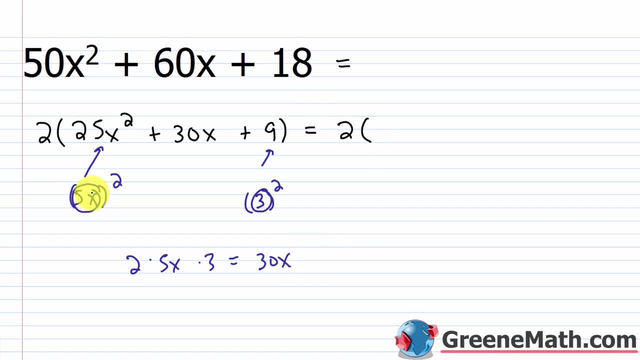 Two times. It's going to be: this guy right here, 5x x plus this guy right here, 3, and this quantity is squared. So whatever is squared here plus whatever is squared here, that quantity is squared. Very easy to set up once you know that you have. 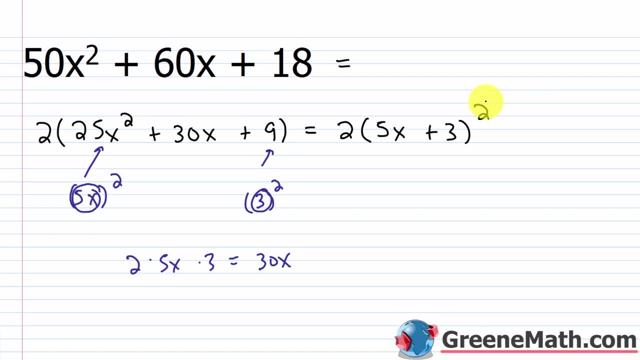 a perfect squared trinomial. So again, we get two times the quantity, 5x plus 3 squared. Now let's take a look at another one. So we have 49n to the fourth power minus 42n squared plus 9.. So the 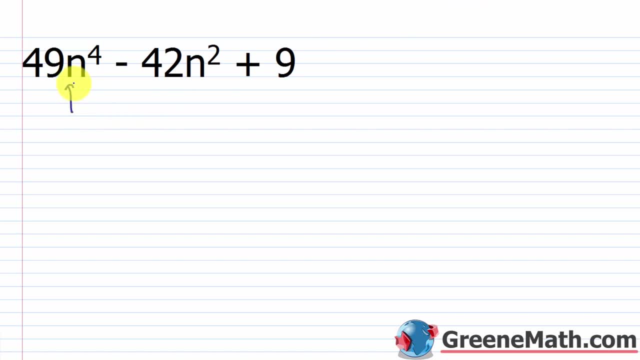 first thing I'm going to look at is the n's. So 49n to the fourth power, I know 49 is a perfect square: it's 7 squared. I know n to the fourth power is a perfect square, it's n squared squared. 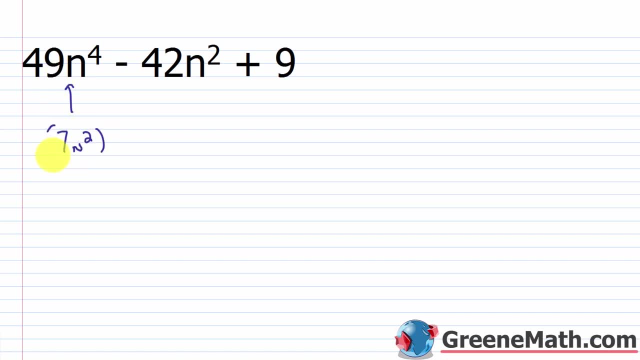 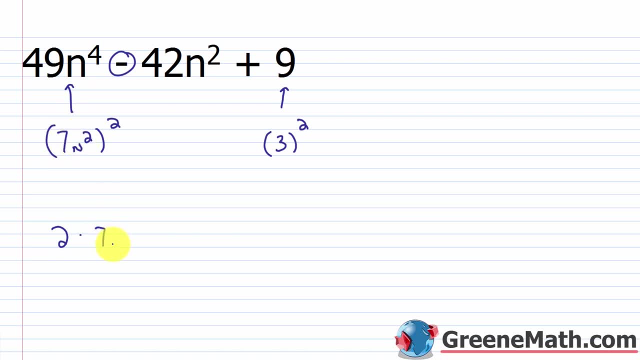 times this right here, 7n squared. times this right here, 3 equal to 42n squared. Forget about the negative. So 2 times 7 is 14.. 14 times 3 is 42.. 42 times n squared is 42n squared, So that's good. 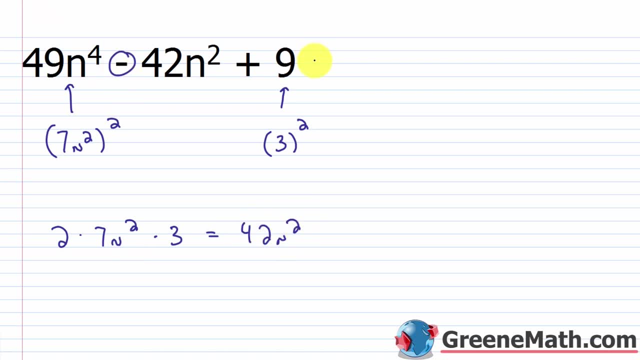 to go there. You just need to remember the minus sign. So with this formula, when I factor, I have something minus, something squared, And what it is is: this is first term here that was squared, Which is 7n squared minus because of the minus sign here, the last term that's squared In this: 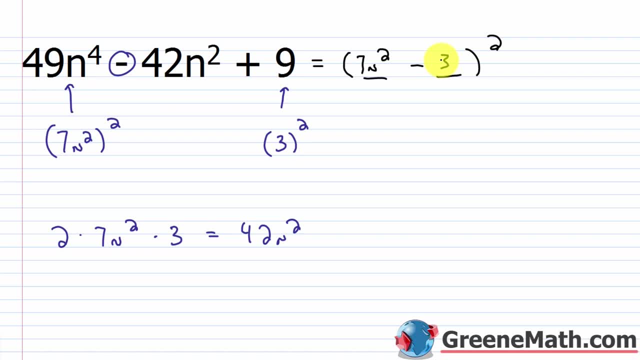 case, that's 3.. So you get the quantity 7n squared minus 3 and this is squared. All right, let's take a look at another one. So we have 9x squared minus 24x, plus 16 minus y squared. So you might look at: 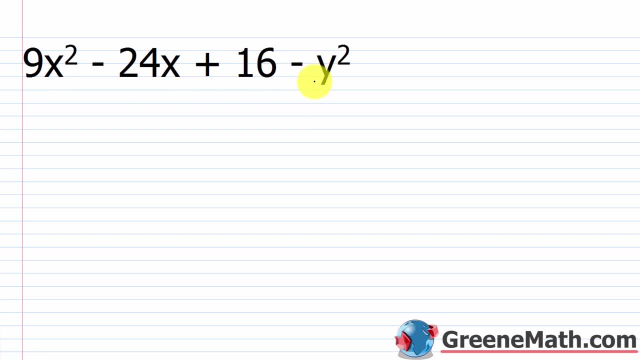 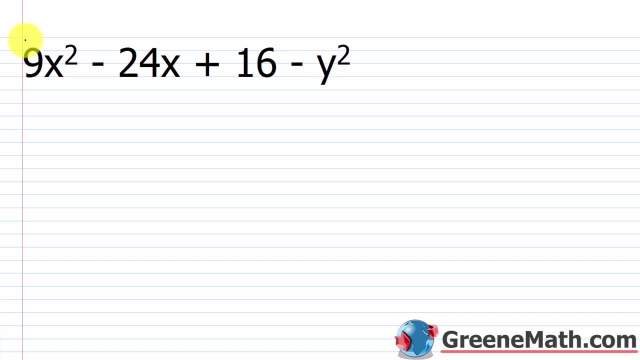 show you this to you, because you probably won't see it right away If I was to enclose this part only inside of parentheses. Let's say: we have the quantity 9x squared minus 24x plus 16, then minus y squared. Now I can factor this because this part right here is a perfect 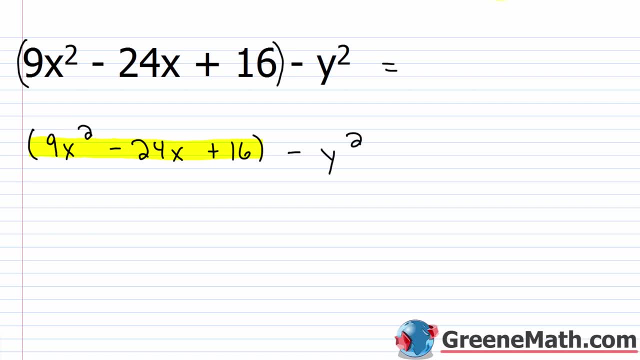 square trinomial. So let's go ahead and factor this: This is 9x squared, So this I could write 3x squared. This is 16, so that's 4 squared. And then for the middle, I have 3x times 4, which is 12x. 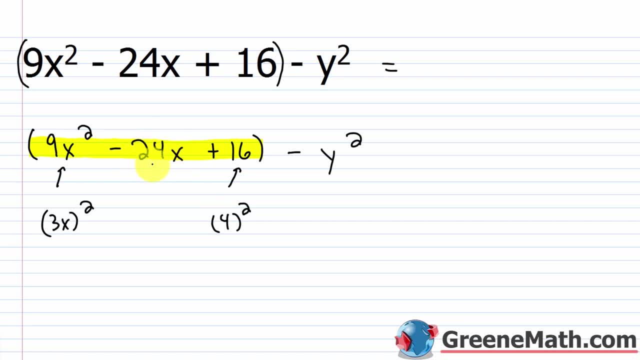 times 2, which is 24x, So that matches up. So all I need to do is say that I have what? 3x this guy right here. I have a minus right there, so minus. and then 4- this guy right here, So the quantity. 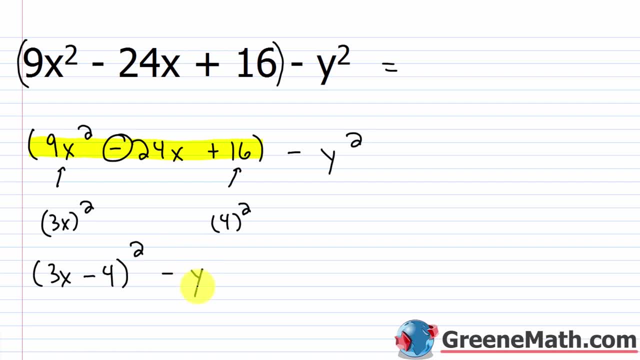 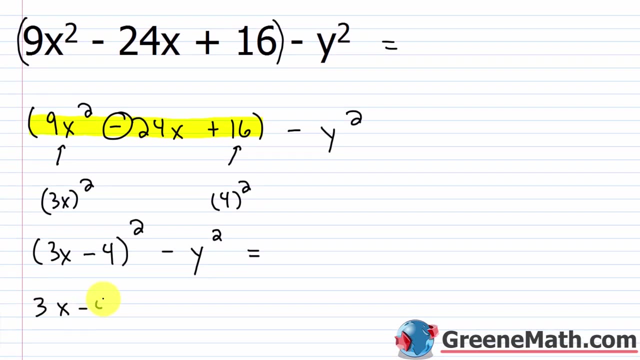 3x minus 4 squared minus y squared. Now what do I have here? I have the difference of two squares. I have something squared minus something else squared. So let's further factor this into the quantity 3x minus 4 plus y times the quantity 3x minus 4 minus y. Now if you go back and you multiply these together, 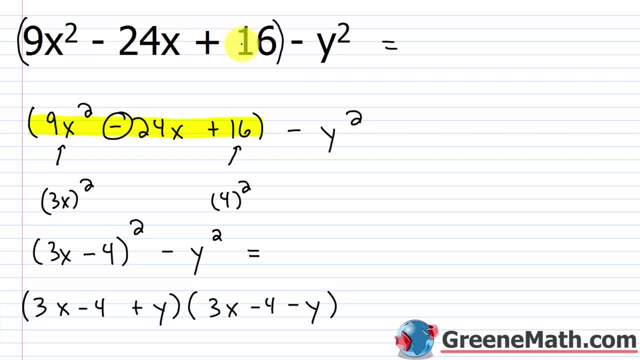 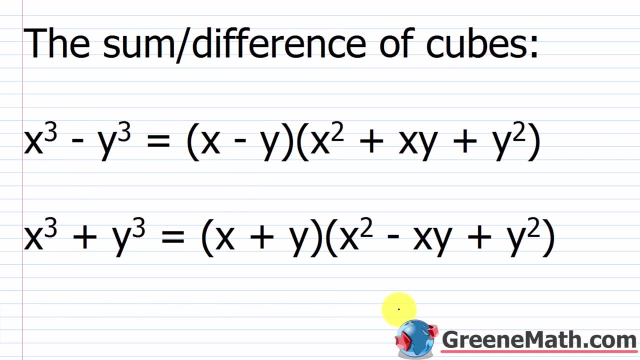 you will end up with 9x squared minus 24x, plus 16 minus y squared. Alright, for the final section. we want to talk about the sum or difference of cubes, So something like the difference of cubes. you have x cubed minus y cubed, So this is going to factor into. 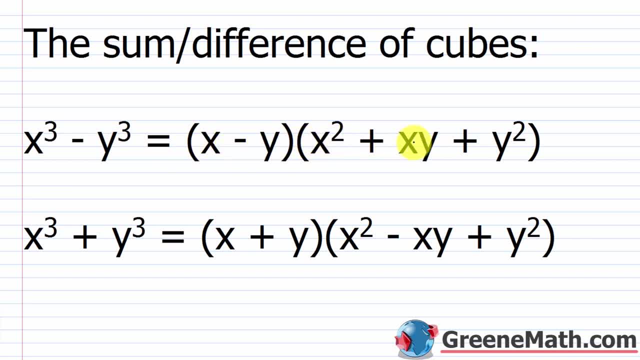 the quantity x minus y times the quantity x squared plus xy plus y squared. So the main thing to remember here is that if you have a negative here, the first sign you see is going to be negative With the sum of cubes. you have x cubed plus y cubed. Everything is the same except 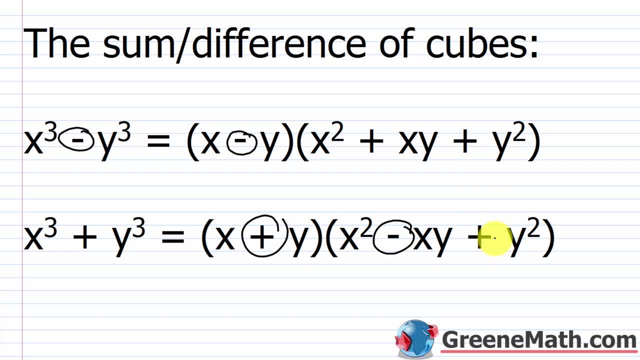 that the first sign is always plus in either. So the way I always remember this is that the first sign is always going to match, the second sign is not going to match and the last sign is always positive. So in other words, if this is minus, this is minus flip. 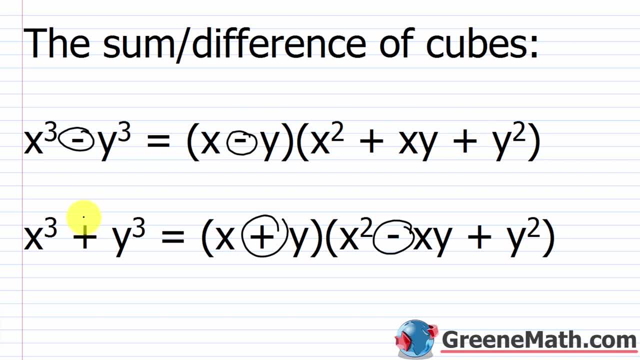 the sign: it's plus, this is always plus. If this is plus, this is going to match, so it's plus. flip the sign because it's not going to match, it's minus, and then this is always plus. So that's how I personally remember it. Now for this part, right. 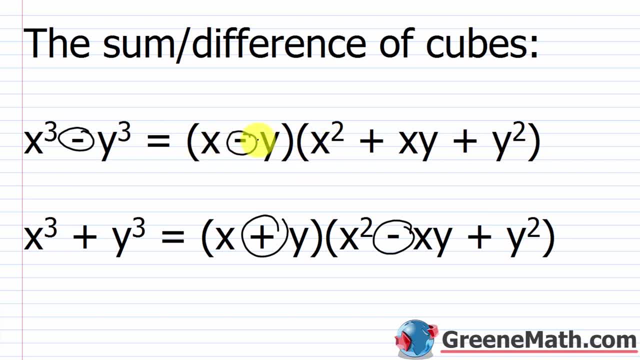 here the multiplication is pretty easy. You just have an x and a y and you have a squared and squared at the end and xy in the middle. So not too hard to memorize that. It's just something you have to practice over and, over and over again and then you know 15 or 20. 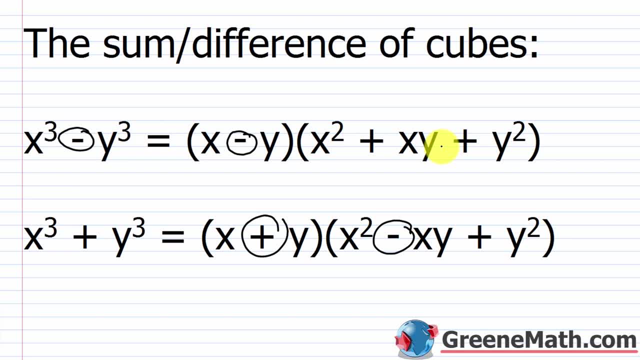 of these. you pretty much have it down packed. but I can tell you, unless you do a lot of problems, you know over time it's something that you will forget and have to revisit. So let's take a look at some examples. Alright, so let's say you had something like negative. 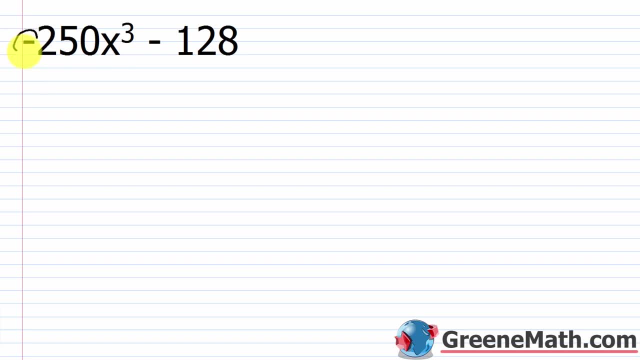 250 x cubed, minus x squared, plus 15 x squared, minus 20 x squared, minus 15 x squared, minus minus 128. so forget about the negative for a second. is 250 a perfect cube? no, it is not okay, and if you didn't know that off the top of your head, you could factor it and figure out that it's. 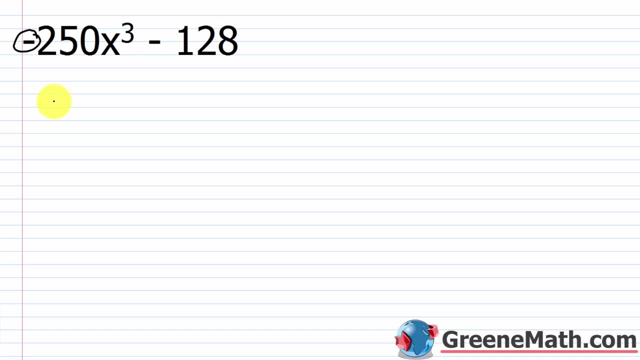 not, but a lot of you will see right away that what you could pull out a 2 and you would have 125, which is a perfect cube. you could pull out a 2 from here and you'd have 64, which is a perfect cube. so a lot of these problems are just going to set up nicely for you. so instead of just pulling, 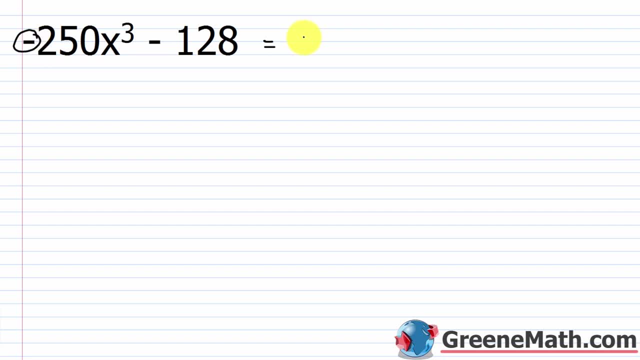 out a 2. let's pull out a negative 2. make it easier on our shell. so we'll pull out a negative 2 and we'll be left with 125 x cubed plus because i'm pulling out a negative 64. let's rewrite this: 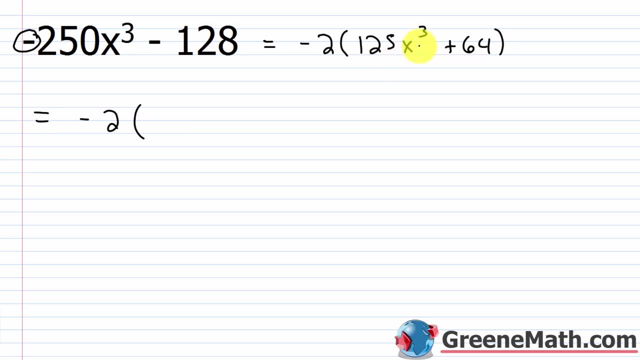 down here. we're going to put negative 2 times the quantity 125 x cubed. 125 is what it's: 5 cubed, x cubed is x cubed. so let's write 5x and that is going to be cubed. then plus you have 64. 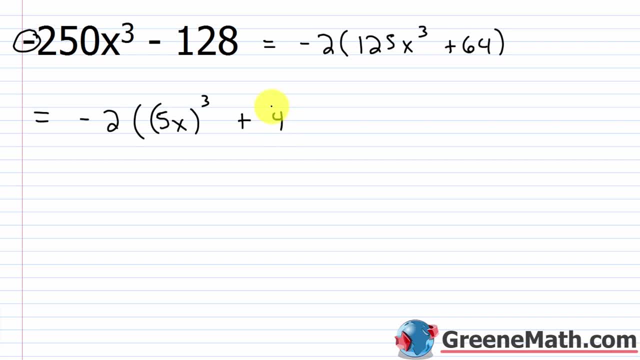 you, 64 is what it's: 4 cubed, 4 cubed, all right. so how do we take this part right here, which is the sum of cubes, and factor it, let's put our negative 2 out in front, and then we know we're going to have. 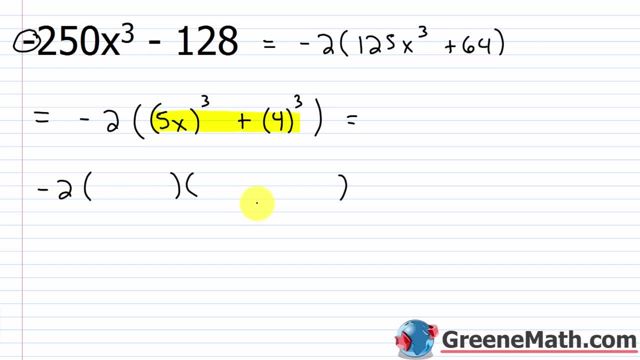 a binomial and a trinomial, so hopefully you can remember that. so remember it was: the first sign is the same, so this will be plus. the second sign you see is flipped, so that means this one's going to be minus and the last one is always plus. now this position here and here is going to match this. 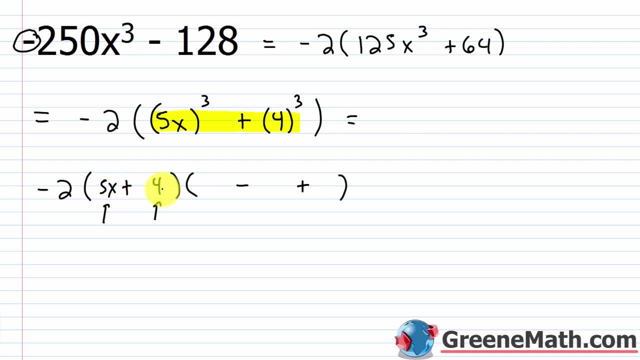 and this right. so it's just 5x and it's 4. so that's easy to remember this position here and here it's going to be the first position squared and the last position squared. so 5x squared would be 25x squared, then 4 squared would be 16. so that's done. the middle part is going to be the. 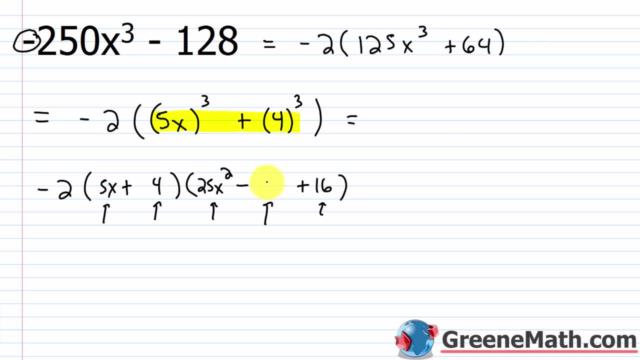 middle part is just this: times this, 5x times 4, would be 20x. so what we end up with is negative: 2 times the quantity 5x plus 4 times the quantity 25x, squared minus 20x plus 16, all right for the. 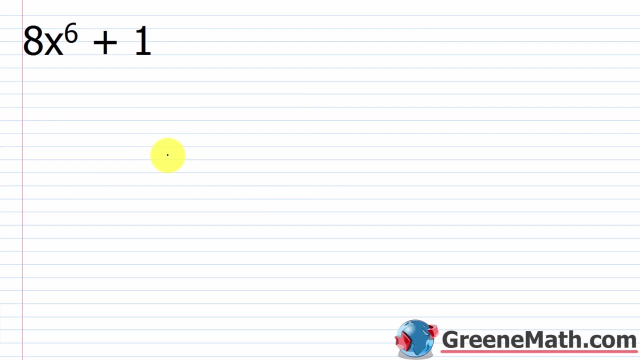 next one. i have 8x to the 6th power plus 1. so do i have a perfect cube here? do i have a perfect cube here? well, yeah, 8 is 2 cubed, then x to the 6th power. i could write as x squared cubed. so let's. 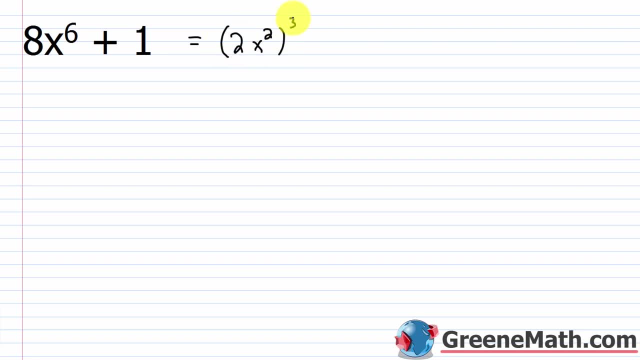 put this all in parentheses and raise it to the third power and then we have plus, we have 1, which is a perfect cube. right 1 to the third power is just 1. so now that i have this in this format, i can factor it very easily. i know that again, let's set up our parentheses, so i've got a binomial here. 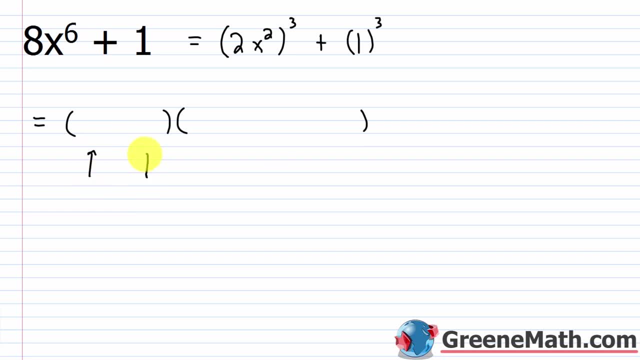 and a trinomial here. so i know this position, and this position is very easy. it's: the first goes first, last goes last. so i have 2x squared and i have 1. very simple. now what sign do i want? remember, if this is plus, the first sign is the same. 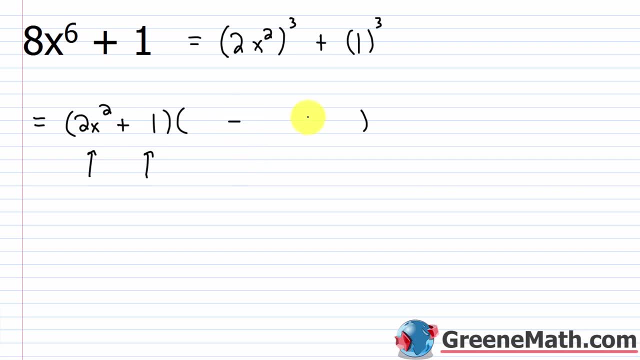 the second sign is different. so plus, minus, the last sign is always plus. very easy way to remember that. now, what goes here and here? well, it's this: squared the first thing, squared goes in the first position. so if i squared 2, i'd have 4. if i squared x, squared x would say the same 2 times: 2 is 4. so 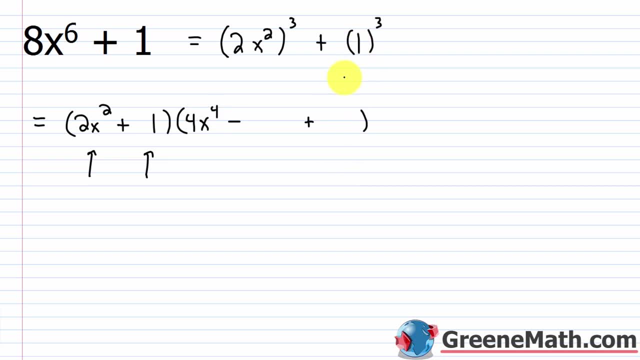 this is 4x to the 4th power. so then the same thing goes here. i want 1 squared. 1 squared is just one. now what goes in the middle is this: times this, 2x squared, times 1 is just 2x squared. so i end up with a quantity 2x squared plus 1. 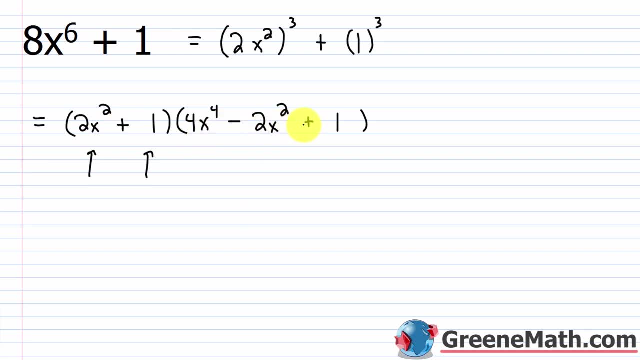 times the quantity 4x to the 4th power minus 2x squared plus 1. let's take a look at one final problem. so we have m to the ninth power minus 343, so m to the ninth power. that's easy, i could. 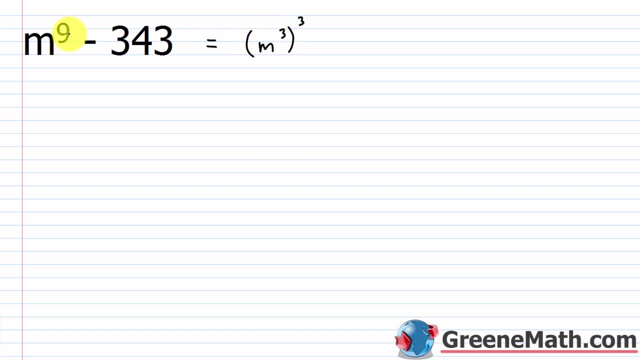 All I have to do with exponents. if I look at an exponent of nine and I want to have something cubed, just divide nine by three. Nine divided by three is three. Because I know when I use my rules of exponents: if I raise a power to another power, I'm multiplying. 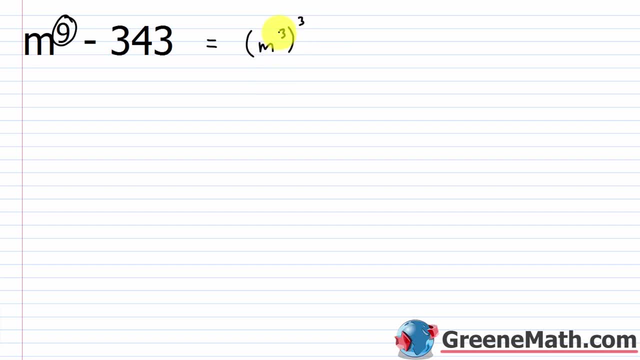 So I can just say: well, if I'm taking m cubed and I raise it to the third power, m stays the same. three times three is none, Then minus, And then what about 343?? Well, that's going to be seven cubed. 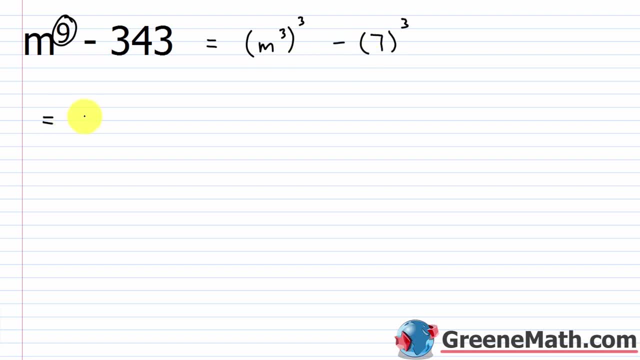 So I've got the difference of two cubes. So what I'm going to do again. let's set this up: You've got a binomial and then you've got a trinomial. The first sign is the same, the second sign is different and the last sign is always. 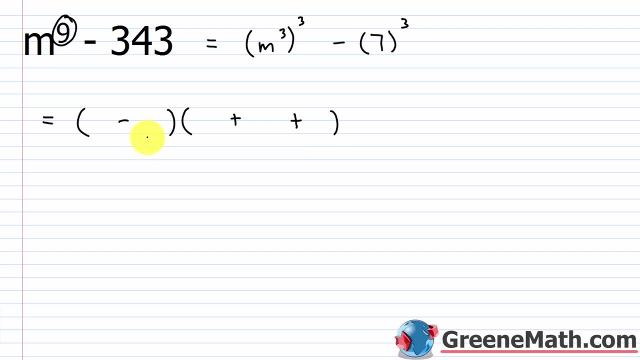 positive. So the first position of each is easy. I want the first position here to be the first position here. I want the second position or the last position here to be the last position here. That's done. Then I want to take the first thing and square it. 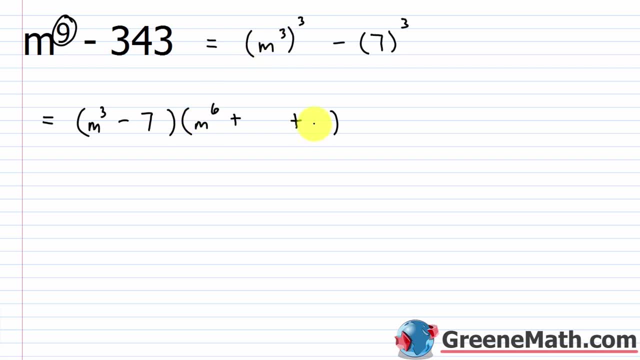 m cubed squared is m to the sixth power. Then what's going to go here? I'm going to take the last thing and square it. Seven squared is 49.. In the middle I multiply the two together, So m cubed times seven is seven m cubed. 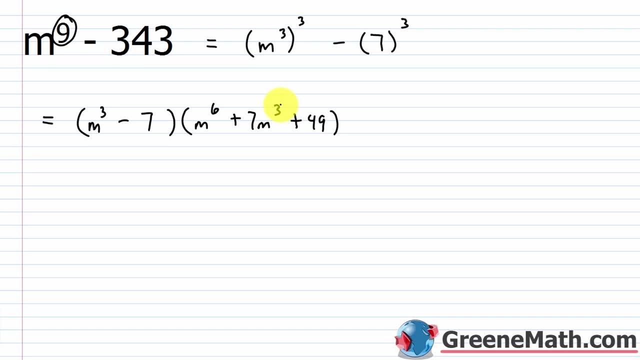 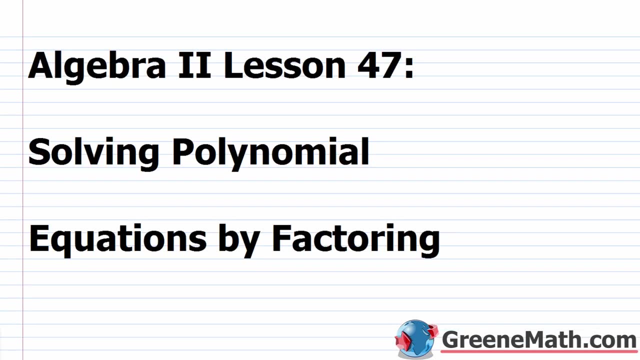 So I end up with a quantity m cubed minus seven times a quantity m to the sixth power plus seven m cubed plus 49.. Hello and welcome to Algebra 2, Lesson 47.. In this video we're going to learn about solving polynomial equations by factor. 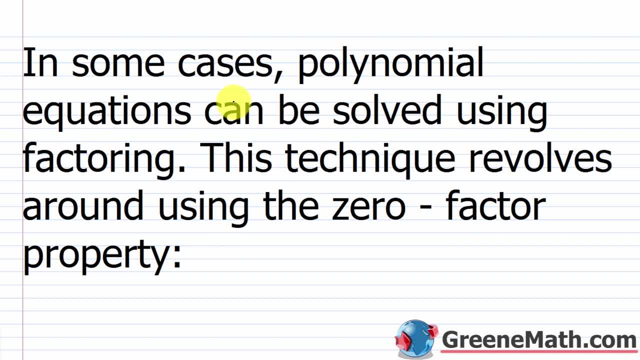 So in some cases, polynomial equations can be solved using factoring. This technique revolves around using the zero factor property. Let me highlight that this zero factor property. Now your textbook might refer to this as the zero product property, but either way, whether 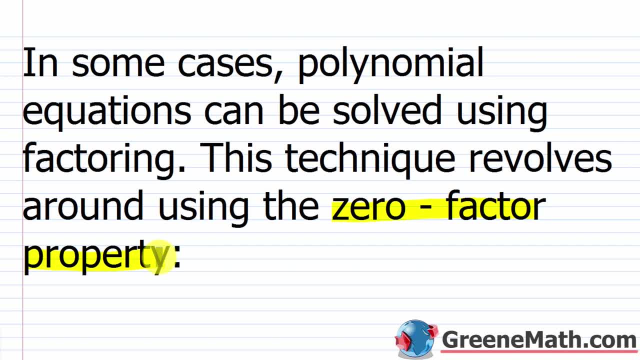 you know it as the zero factor property or the zero product property. it's important for you to understand what it means. So here's an explanation of the zero factor property. So here's an explanation of the zero factor property. So here's an explanation of the zero factor property. 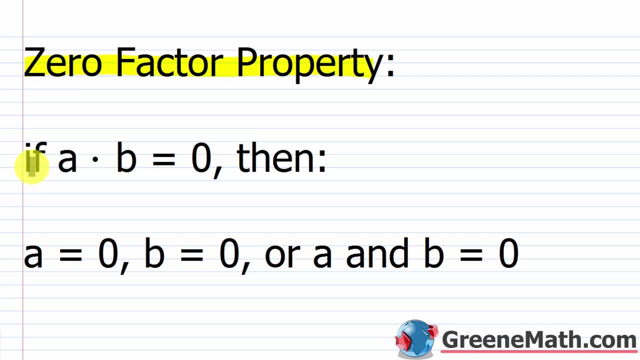 Let me highlight this: You have if a times b equals zero. So let's stop for a second. A is just some unknown, b is some unknown, So this could be x times y, it could be z times q. It could be presented in any different way. 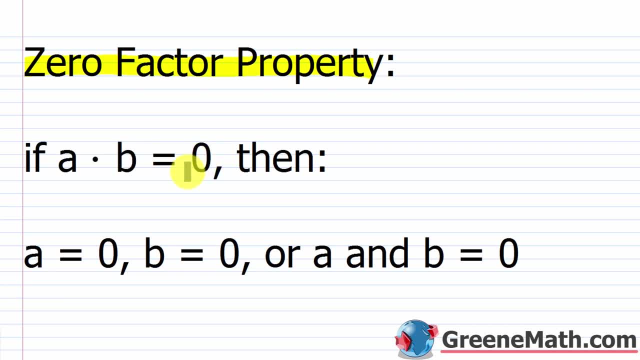 Two unknowns are multiplied together and the result is zero. If we have that, then one of the following scenarios has to be true, based on the fact that if I multiply something by zero, I get zero, I get zero, I get zero. 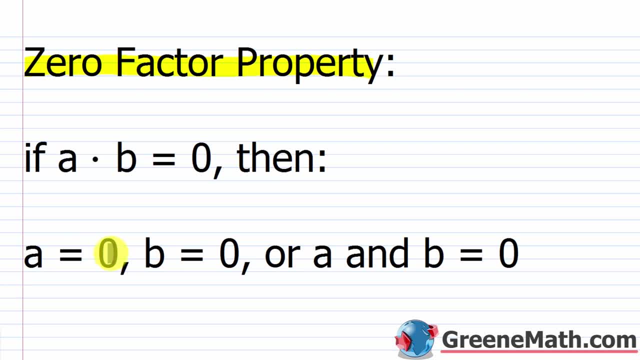 So it could be that a is 0 and b is not 0.. So, in other words, 0 times something that's not 0 would give me 0. It could be that b is equal to 0 and a is not 0. 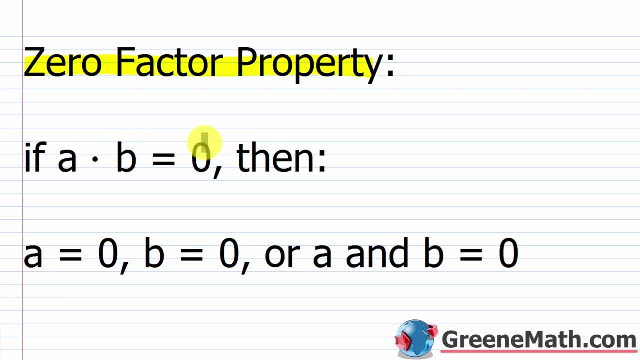 So something that's not 0 times 0 would give me 0. Or the third and final possibility could be that a and b are both equal to 0.. 0 times 0 would also give me 0. So this is very important to understand. 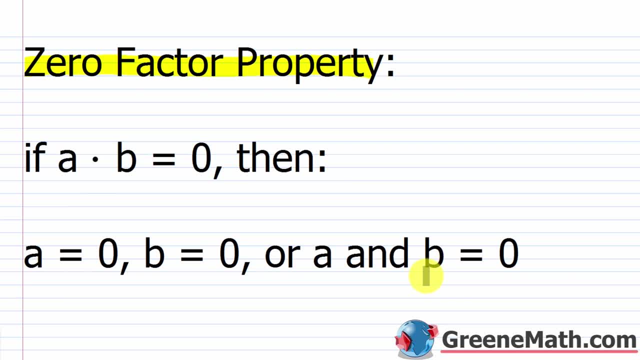 And when we start solving these equations using this property, it's not going to look like this, It's going to look slightly different, And I'm going to refer back to the zero factor property. And you go: oh yeah, that makes sense now. 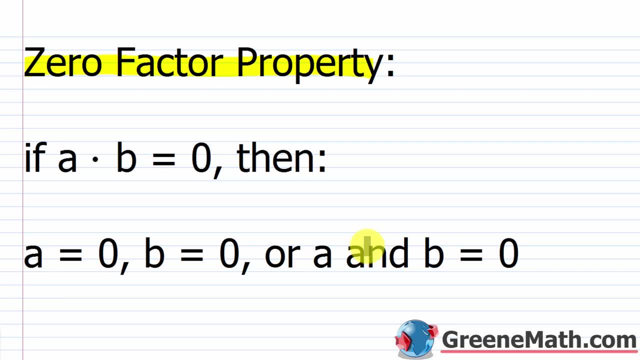 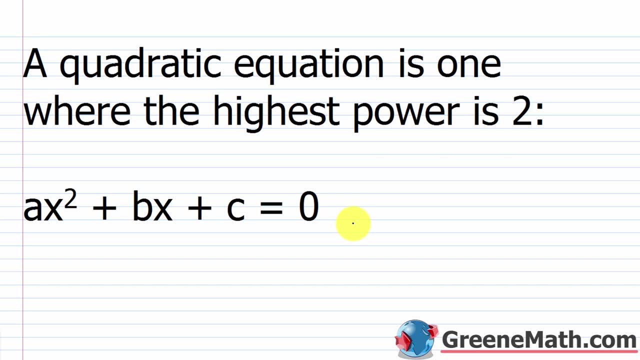 But it's very important that you understand this conceptually. That way, when we start working through the exercises, you understand what's going on. All right, so the focus for today is going to be to solve quadratic equations by factoring. We did this back in Algebra 1.. 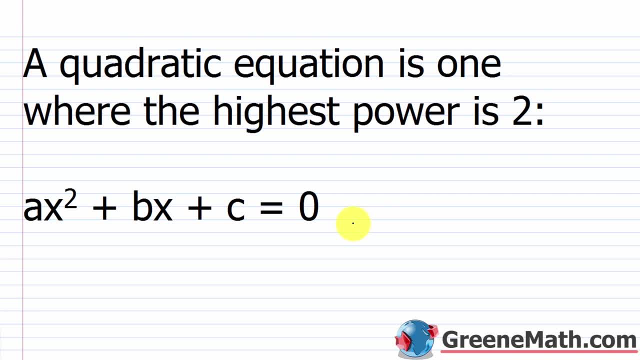 And then most of you will recall that some of these we couldn't factor. And when we had something that we couldn't factor, we learned later on in Algebra 1 we could use something known as completing the square, Or we also can use the quadratic formula. 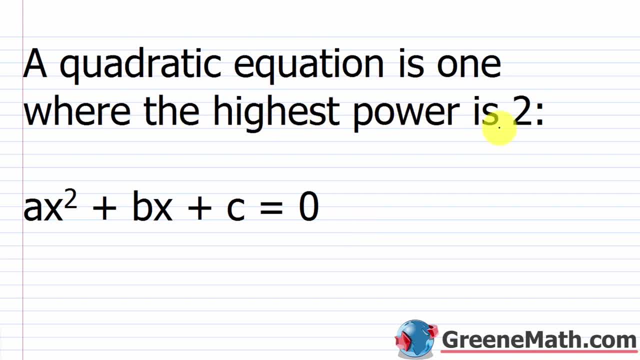 So a quadratic equation is one where the highest power is 2.. So, in other words, if I see something like ax squared plus bx plus c equals 0, you look at your exponents, This one's a 2.. This one's obviously a 1.. 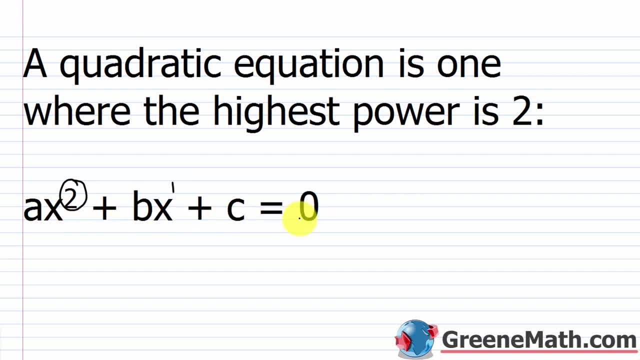 And so the highest exponent is a, 2. So this is a quadratic equation. Now, with your quadratic equation you have a as the coefficient for the squared variable, b is the coefficient for the variable raised to the first power and c is the constant. 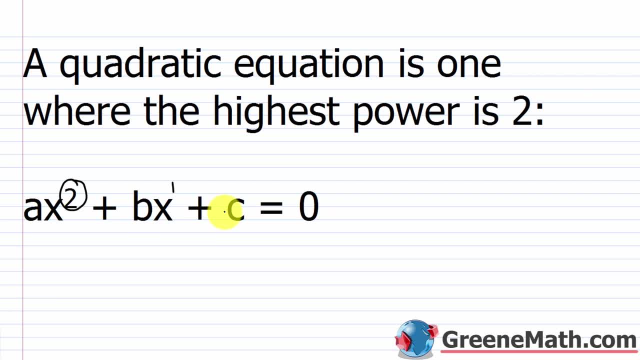 a, b and c can be any real number, with the one exception that a is not allowed to be 0, because you obviously wouldn't have a quadratic equation anymore. If I had 0 times x squared, that's just 0. And in that case I have: bx plus c equals 0.. 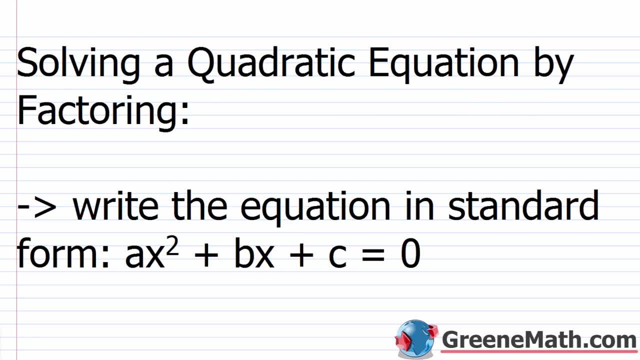 That would be a linear equation now. So let's talk a little bit about the steps that we would use to solve a quadratic equation. Now, if you get something that's more advanced than a quadratic equation and it's factorable, you're basically going to use the same steps. 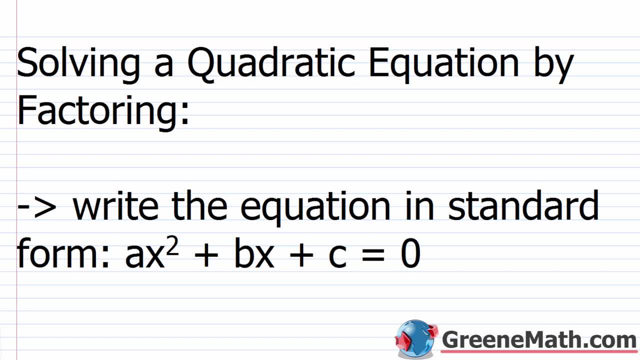 You might see something with the highest power being a 3 or 4 or 6.. And there might be some tricks that you can use. You might be able to factor using substitution. You might be able to factor using grouping. There's all kinds of scenarios where this will be beneficial for you. 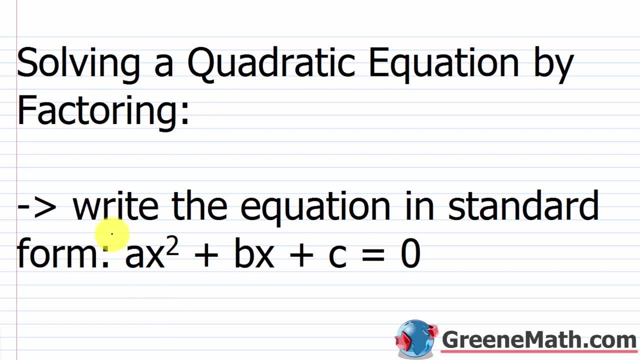 So solving a quadratic equation by factoring, the first thing you want to do is write the equation in standard form. So standard form: we've talked about a lot. So the left side over here we have ax squared plus bx plus c. 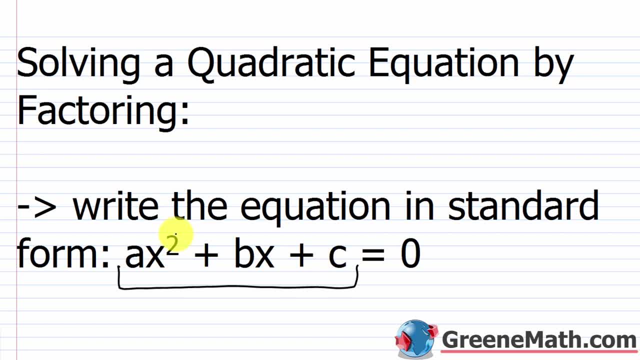 And if I was writing a polynomial in standard form, we know we want it in decreasing order of powers. So I would start with the highest power, which is a 2.. Then I would go to the next highest power, which, in this case, is a 1.. 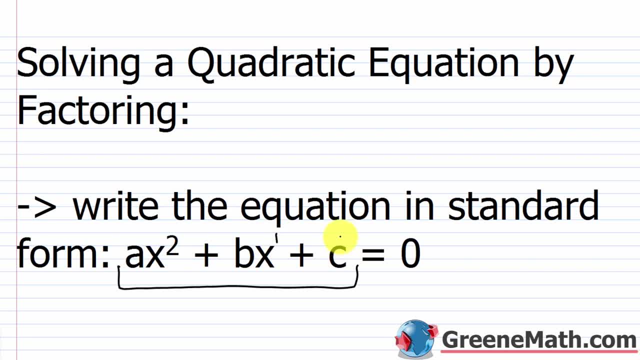 Then I would go to kind of the next highest power, which we have a constant, So we could say that variable is raised to the power of 0. So I'm going to go to the next highest power, which in this case is a 1.. 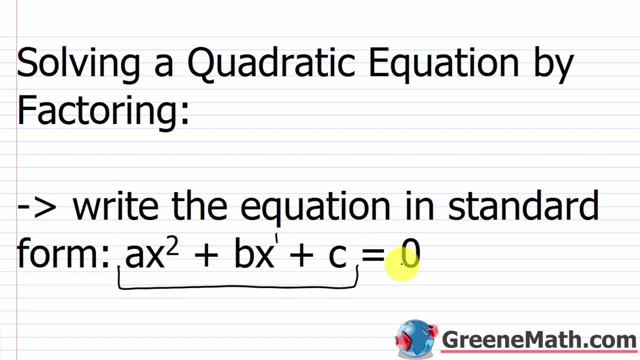 And then I'm going to pick the highest power, which is a 1.. Then I'll say that the highest power is 0. So you'll notice that this is set equal to 0. And this is so we can use our zero factor property. 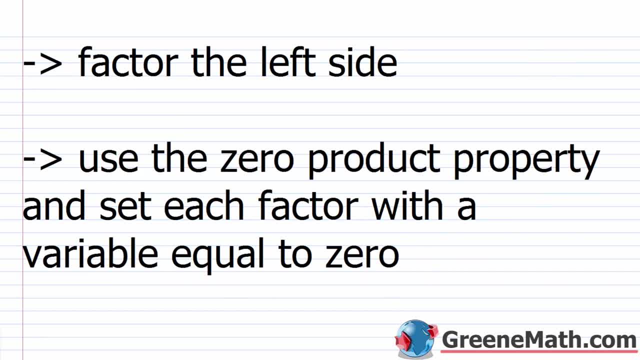 We want this to be zero, Alright. so the next step is to factor the left side. You've got a trinomial on the left side. You've got zero on the right, So you factor the left side. That's going to put it into the product of two binomials. 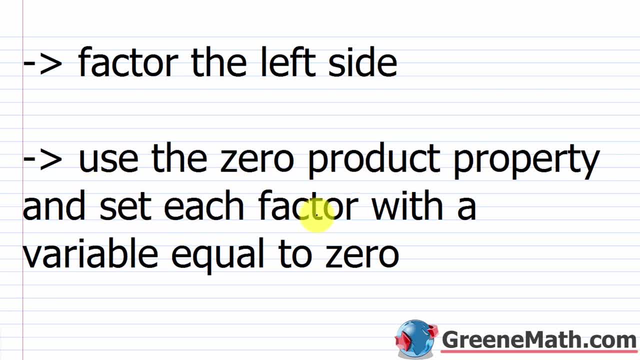 Then we're going to use the zero product property and set each factor with a variable equal to zero. And the reason we say: with a variable, sometimes you can pull something else out, okay, before you start factoring, and you don't need to set that equal to zero, because that would. 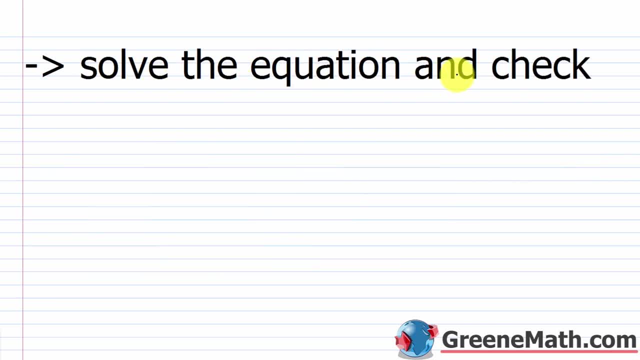 be irrelevant, All right. the last thing is obvious. You just want to solve the equation and check, All right. so let's get started with the first example. So we have x squared minus 12x equals negative 36.. So the very first thing I want to do is put this in standard form. 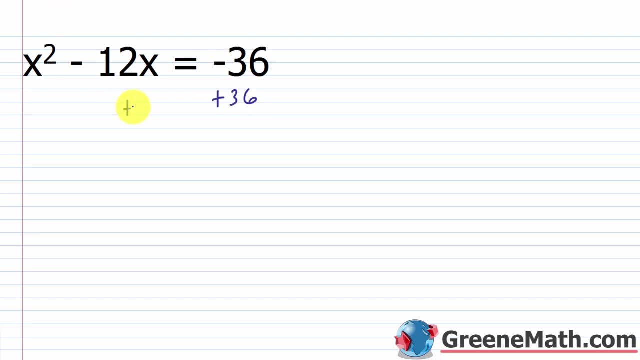 So all I need to do is add 36 to both sides of the equation, So I would have x squared minus 12x plus 36 is equal to negative. 36 plus 36 is zero. So the left side. if you look at it, this is a trinomial in standard form. 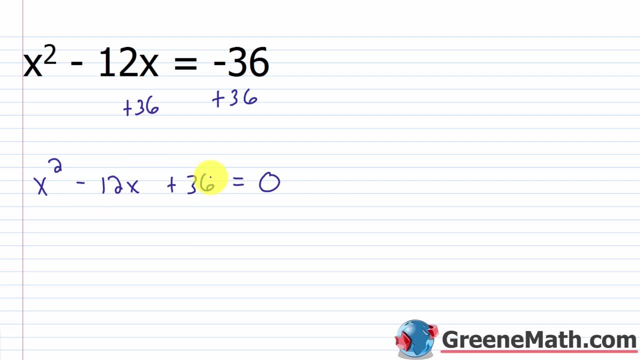 I've got x squared, x to the first power and I've got my constant. Okay, so that's what I want. On the right side, I have a zero. So what I want to do now is I want to factor this left side into the product of two binomials. 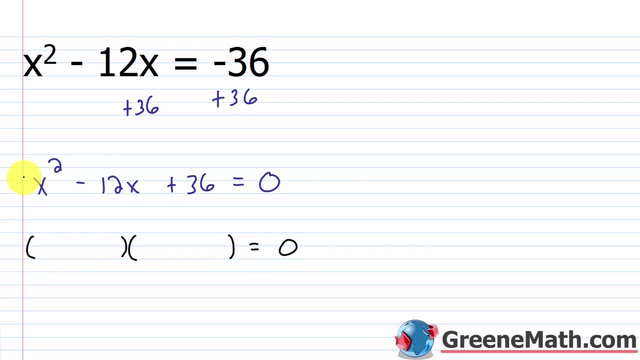 Very easy to do. I know that I have x squared here and this is a one as the coefficient for x squared. So this would be x and this would be x, And I simply need to find two integers whose sum is negative 12 and whose product is 36.. 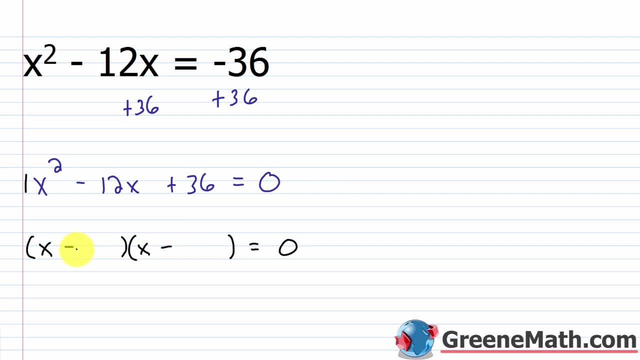 Well, I know I'm looking for a negative and another negative. Negative plus negative is negative. Negative times negative is positive. Okay, so let's just think about factors of 36.. I've got 1 and 36.. I've got 2 and 18.. 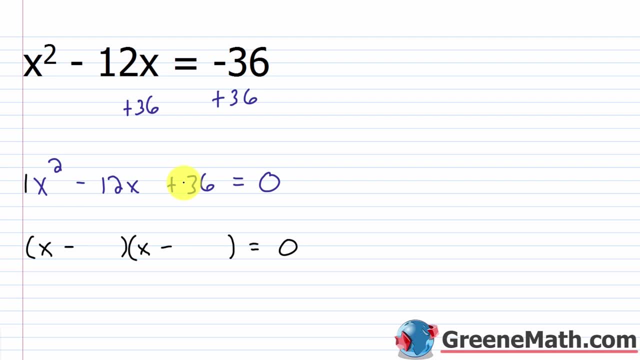 I've got 3 and 12.. I've got 4 and 9.. I've got 6 and 6.. Now think about 6 and 6.. 6 plus 6 gives me 12.. So I just need to work out the signs. 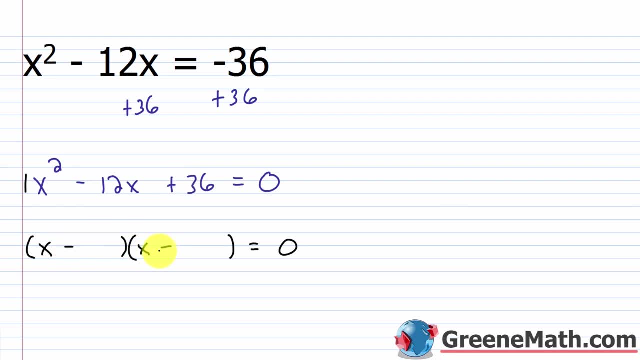 Remember we already figured out it's a negative and a negative. So negative 6 plus negative 6 would give me negative 12.. Negative 6 times negative 6 would give me positive 36.. So x minus 6, that quantity times x minus 6.. 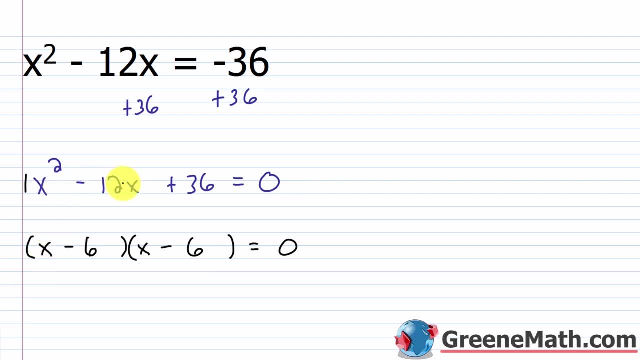 Now you'll notice that essentially, we could have found this by using our special factoring. This is a perfect square, x squared, and 36 is a perfect square. And remember how to check the middle term You think about. is this right here? this 12x, 2 times x, times 6?? 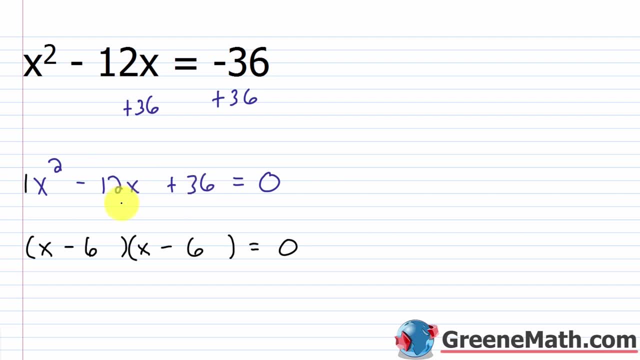 Well, yeah, 2 times 6x is 12x, So we know this would have factored into the quantity x minus 6 squared. Now, in this particular case, because we have the same thing twice, I don't need to set each one equal to 0.. 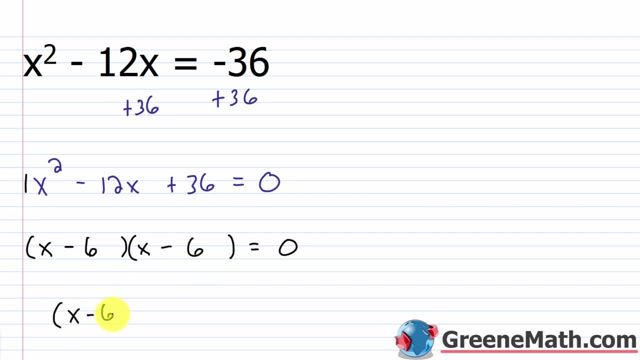 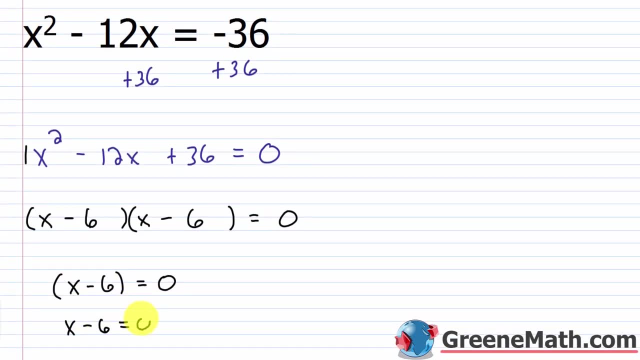 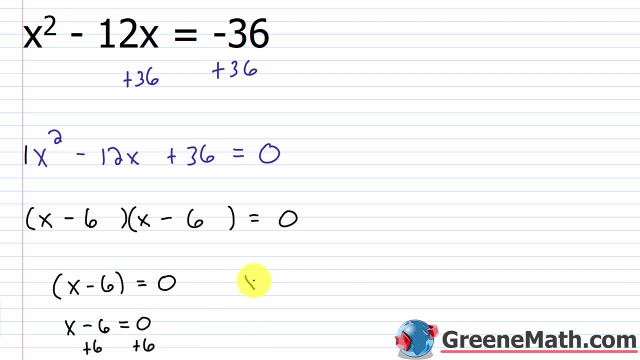 I add 6 to both sides of the equation And I get that x is equal to 6.. Now let me stop and explain what I did. If we consider the 0 factor property- remember, this is multiplication. here- This is multiplication. 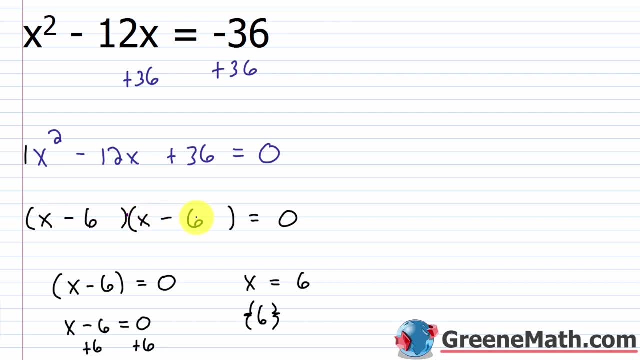 So if the quantity x is equal to 7, x minus 6 is multiplied by the quantity x minus 6, well, one of these- and it happens to be the same thing- has to be 0. So if I can make this equal to 0, then 0 times whatever this is. 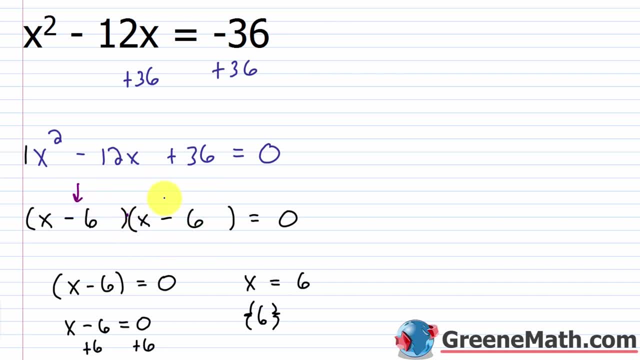 it doesn't matter that it's the same thing. if it was something different, if it's multiplied by this, it would give me 0.. So in other words, if I plugged in a 6 here, 6 minus 6 would be 0,. 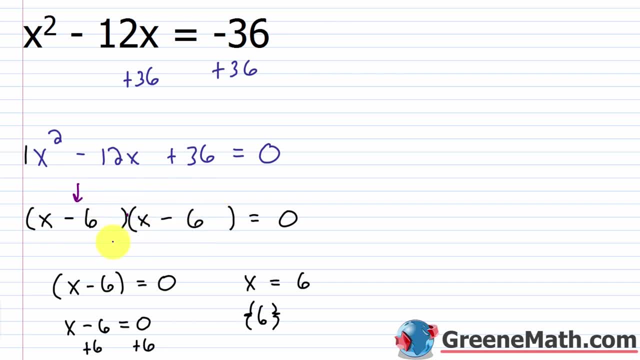 0 times this, whatever it would be- and I know it's the same thing in this case- would give me 0.. So that's how the 0 product property or 0 factor property, however you want to say, it- allows us to solve these equations when they're able to be factored. So if you wanted to, 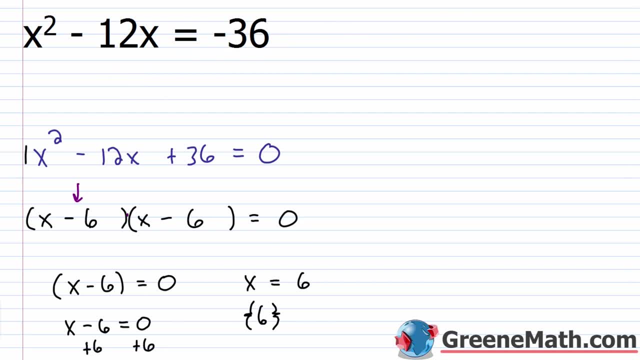 check this. there's only one solution in this case. we'd plug in a 6, everywhere there's an x, So you'd have 6 squared, which is 36,, minus 12 times 6,, which is 72,, and this should equal. 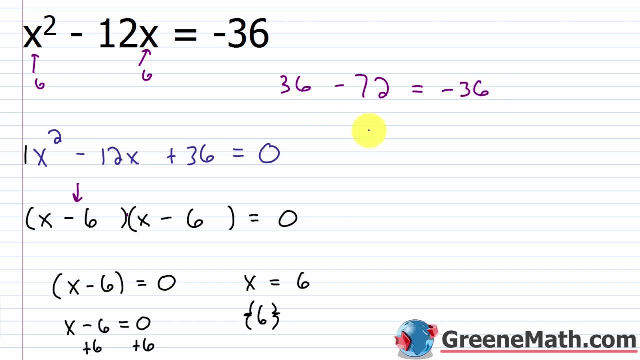 negative 36, and it does. 36 minus 72 is negative 36,, so you get negative 36 equals negative 36.. So this checks out. All right, let's take a look at one that's a little bit more challenging. 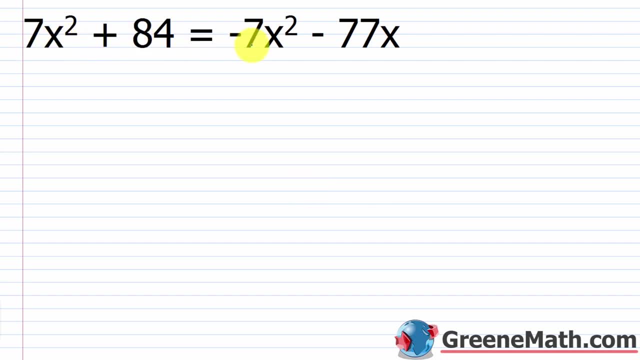 So we have: 7x squared plus 84 is equal to negative, 7x squared minus 77x. So again, I want to put this in standard form. So I'm going to take everything and just move it to the left. the right should be 0.. So I'm going to add 7x squared to both sides of the. 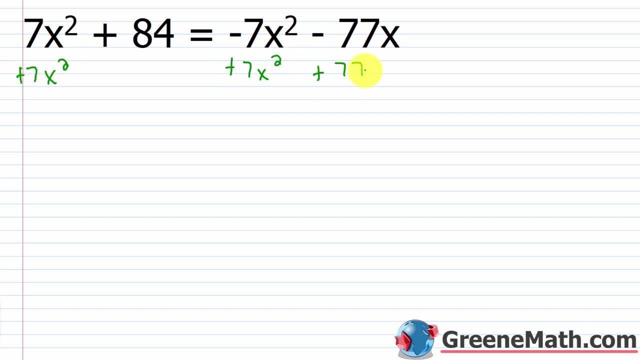 equation and I'm going to add 77x to both sides of the equation equation. So this is going to cancel and become zero. So on the left side I'm going to have 7x squared plus 7x squared, which is 14x squared, then plus 77x, then finally plus 84.. Remember. 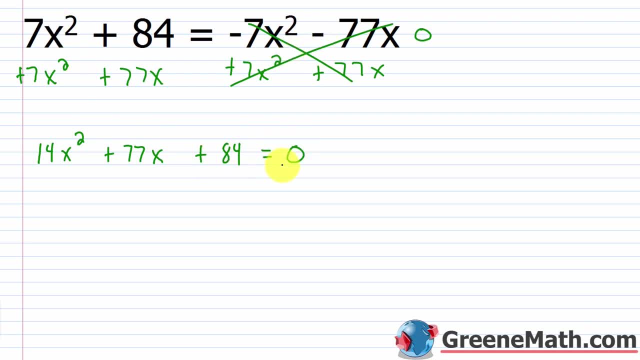 the right side is zero, So this equals zero. Don't forget the equal zero. It's very important that you put equal zero. I see a lot of students forget to put this. they factor it and then they lost their way. They don't know what to do next. All right, so I want to factor this Now. 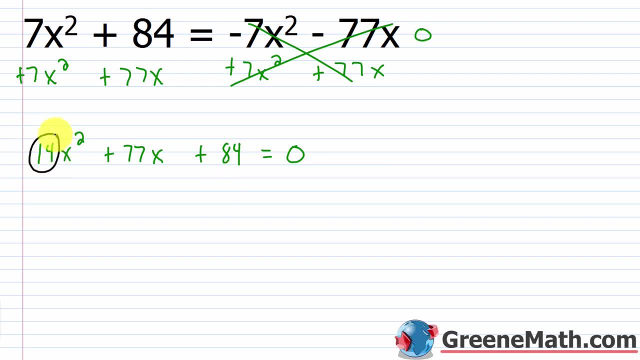 this is the harder scenario where the coefficient here is not a one. So again, you can use reverse FOIL, You can use factoring by grouping. You can basically do whatever you want to do. It's just something that's going to work for you. Now, the first thing you should notice here is that you 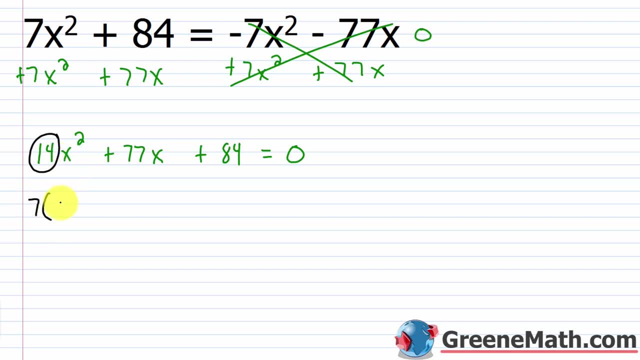 could pull a seven out. So if I pull out a seven, this would be 2x squared plus 11x plus 12.. Instead of 7x squared, I'm going to put 7x squared. So I'm going to put 7x squared plus 11x plus 12.. 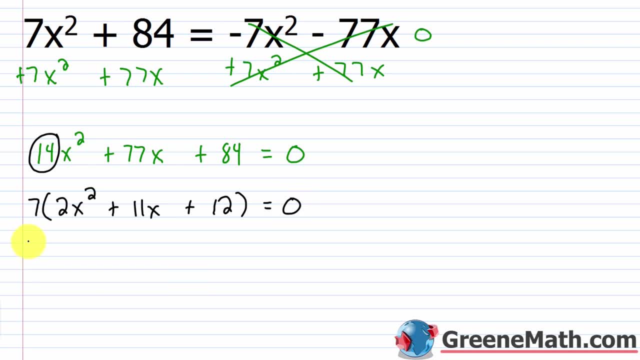 So I'm going to put 7x squared plus 11x plus 12.. Instead of 7x squared, I'm going to put 7x squared plus 11x plus 12.. So I'm going to put 7x squared. inside the parentheses. This is equal to zero, So keep my. 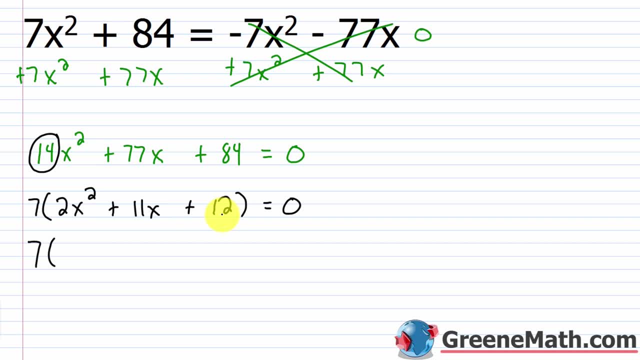 seven outside, and I want to factor this. I'm going to use grouping because it's just a little bit easier for me to do So. what I want to do is find two integers whose product is 2x12 or 24.. So I want the product. 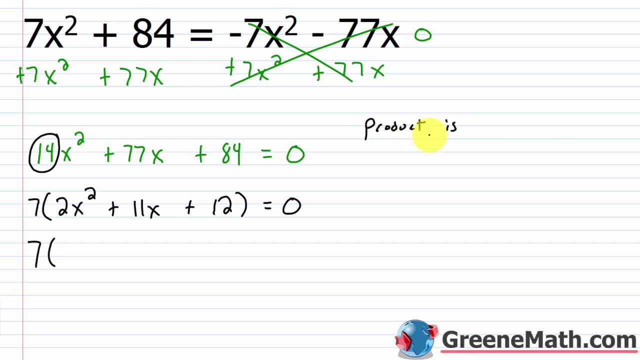 to be 24.. So product is 24.. The sum is this middle coefficient of 11.. So you think about 24, and right away, you think about 3 and 8,. right, 3 plus 8 is 11.. 3 times 8 is 24.. So I could write that middle. 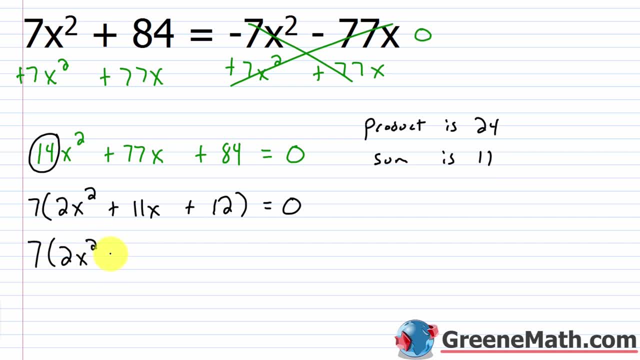 term, We'll have 2x squared. We'll put plus 8x, plus 3x, plus 12.. Again, for those of you who are unfamiliar with this process, all I'm doing is I'm rewriting the middle term using those two. 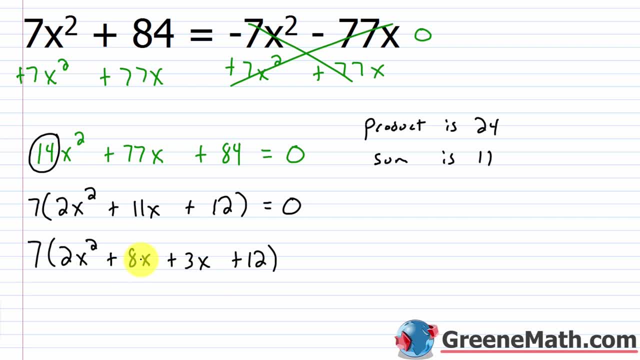 integers that I found. So instead of 11x, I've expanded this to 8x plus 3x. 8x plus 3x is 11x, so it's legal. So let me put equal zero. Now I'm going to factor inside the parentheses using: 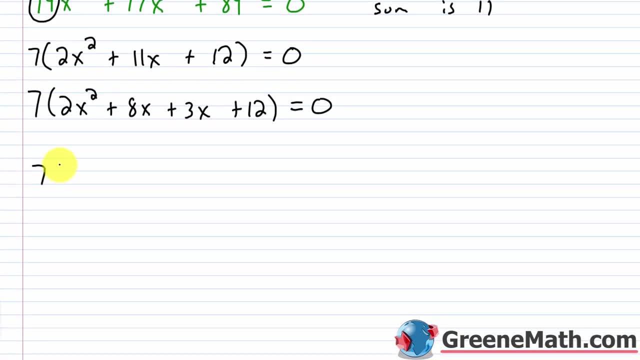 grouping. So this is super easy. We have seven times. From the first group, I'd pull out a 2x. What would be left is x plus 4, then plus. From the second group, I'd pull out a 3.. What would? 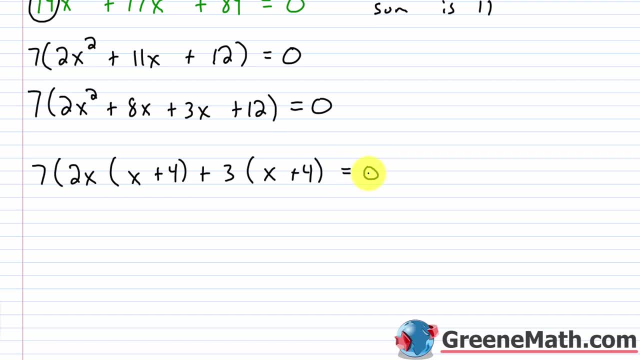 be left is x plus 4.. So you can see you have this common binomial factor here of x plus 4.. So I can factor that out: I would have 7 times the quantity x plus 4, then times the quantity, you'd have 2x. 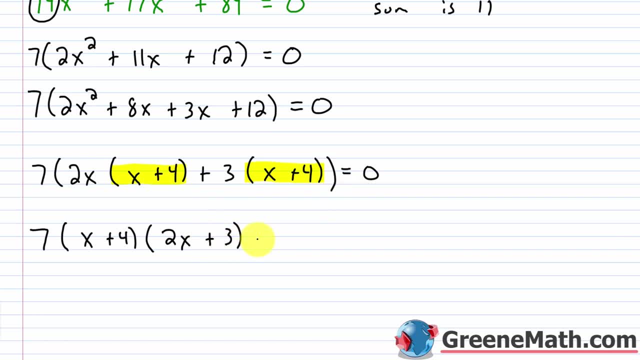 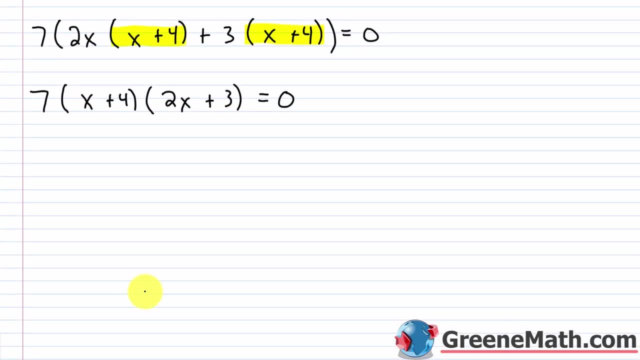 plus 3.. Now, remember, this equals zero. Okay, let's scroll down and get some room going. Now I have three factors here: 7 is multiplied by the quantity x plus 4, which is multiplied by the quantity 2x plus 3.. So three factors. This is a factor. 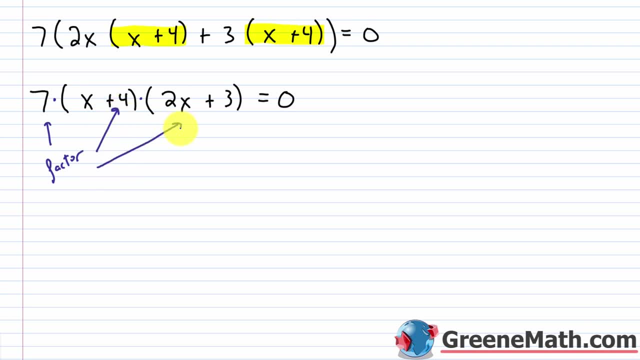 So is this. So is this Now? 7 does not have a variable involved. Do I need to set it equal to zero? No, I'm not going to waste my time. I'm only going to set a factor with a variable equal to. 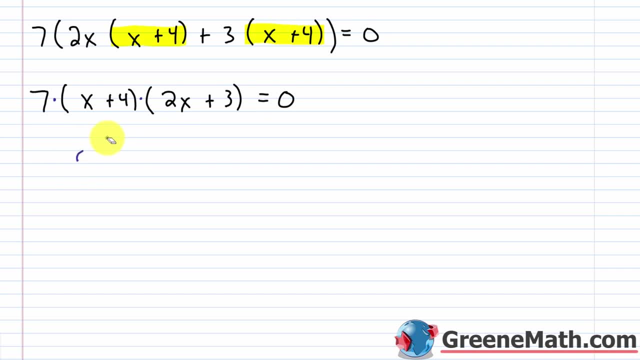 zero. So I'm going to take this quantity, x plus 4, and set it equal to zero. So x plus 4 could be equal to zero, or okay, we'll use this connective word, or 2x plus 3.. 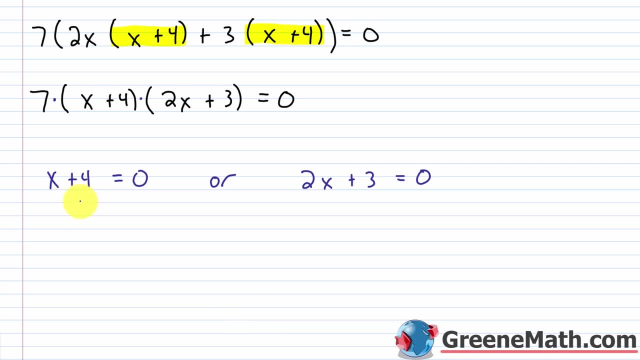 Could be equal to zero, So it could be true that this equals zero or this equals zero. Those are our two scenarios, Because, remember, if a times b equals zero, then either a is zero, b is zero or they're both zero. Okay, so that's what we're just doing here. It's just a little bit more. 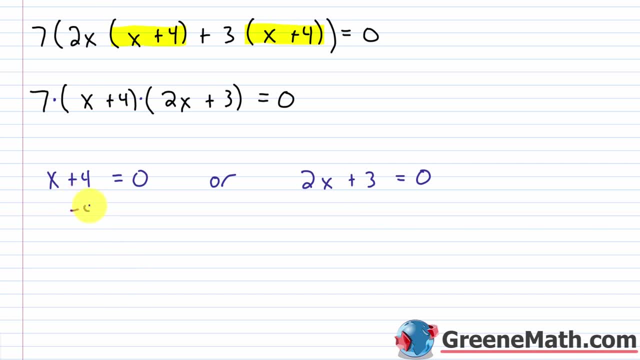 complex, All right. so to solve the first one, I just subtract four away from each side, and I get x is equal to negative four. For the second one, I subtract three away from each side. This cancels. I get 2x is equal to negative three. I divide both sides by two and we end up with x is equal. 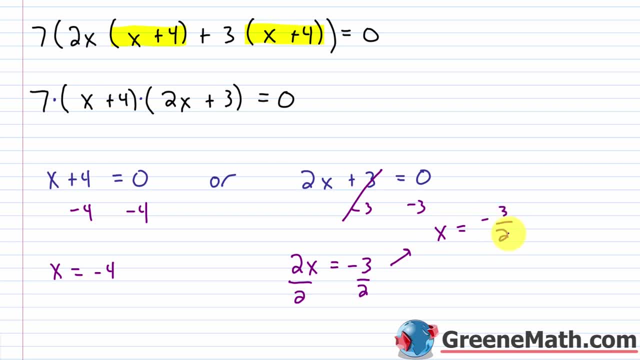 to negative three halves. So in solution set notation, remember we'll put some curly braces. Let's list negative four comma, negative three halves. Those are two solutions and that's it, We're done. If you want to pause the video and check, I would welcome you to do that. I've 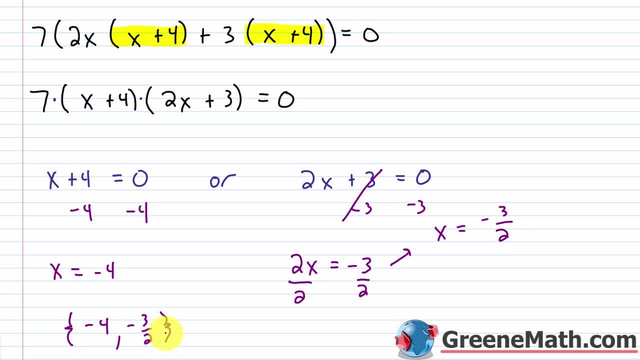 already checked this so I know it works out And in the interest of time I'm not going to check anymore. But all you would need to do is just plug in a negative four for every x in the original equation. You'll verify that the left and the right side are equal. Then you'll plug in a negative three halves and for each x in the original equation. 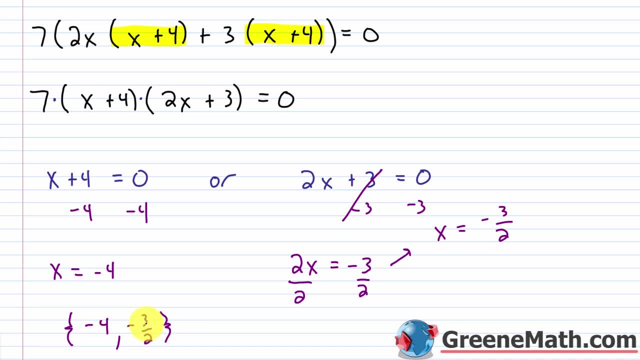 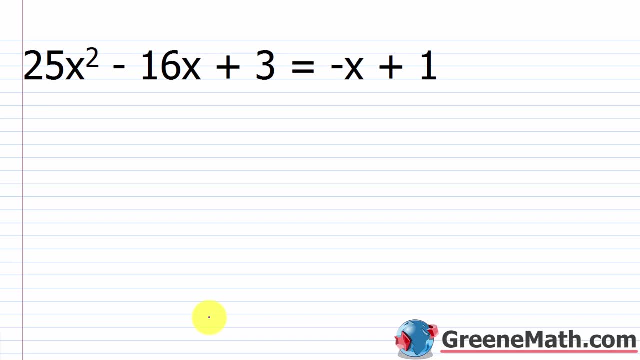 And again you'll verify that the left and the right side are equal. All right, let's take a look at another one. So we have 25x squared minus 16x plus three, and this is equal to negative x plus one. 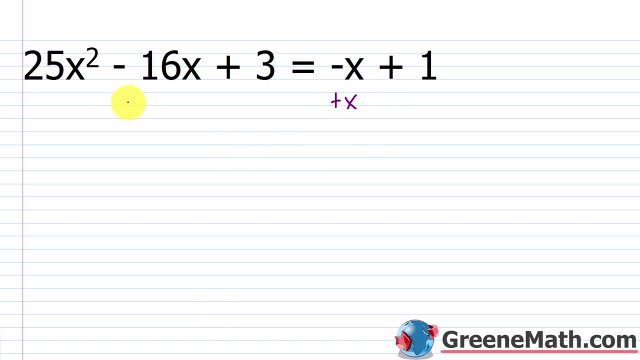 So again, move everything over to the left. So I'm going to add x to both sides of the equation and I'm going to subtract one away from each side of the equation. So the right side has canceled and it is now zero on the left side. 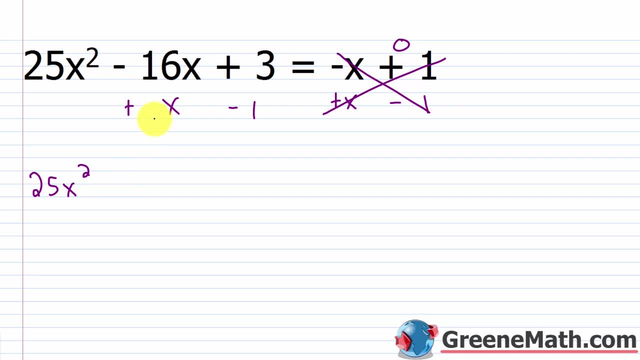 I still have my 25x squared, and then negative 16x plus x. So you could say: plus one x is negative 15x, and then three minus one is two, So plus two, All right, So now this equals zero. 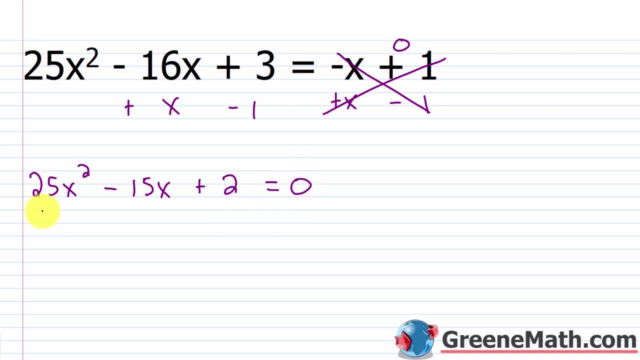 We'll forget that, And the simple fact is there's nothing I can pull. I can stop before I start. This is divisible by five. This is divisible by five and three. This is a two, It's prime. So it's only divisible by two and one. 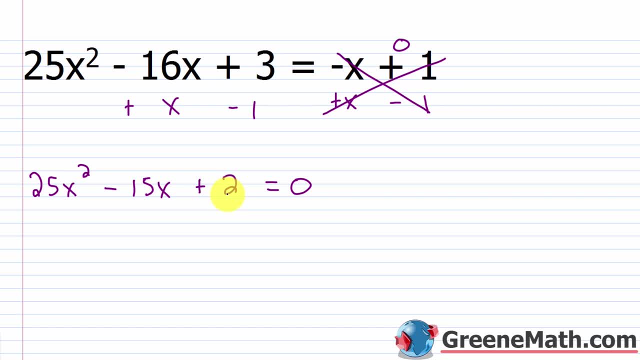 So if I think about what I'm going to do, I'm just going to factor this using grouping: So we want to find two integers whose product is 25 times two or 50. So the product is 50. And then the sum is negative, 15, that middle coefficient. 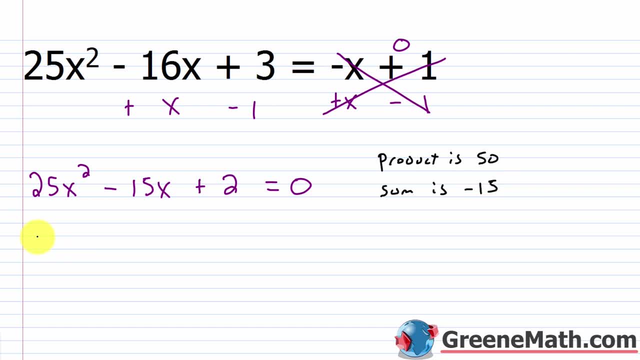 So we think about this. We know that it's going to be a negative and another negative, So go through the factors of 50.. Right away, I think about 10 and five. Negative 10 and negative five would work right. 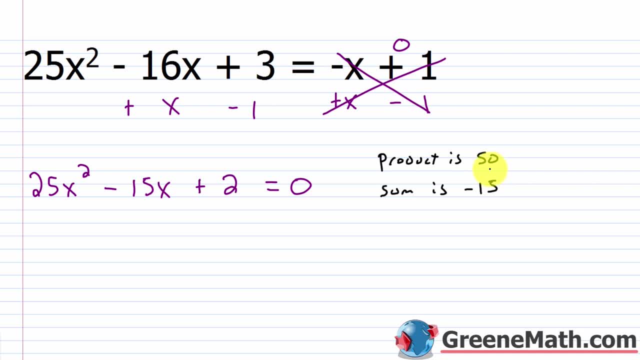 Negative 10 plus negative five is negative 15.. Negative 10 times negative five is positive 50.. So again, I'm going to use that to rewrite this middle term. I'm going to have 25x squared minus 5x, minus 10x plus two, and this equals zero. 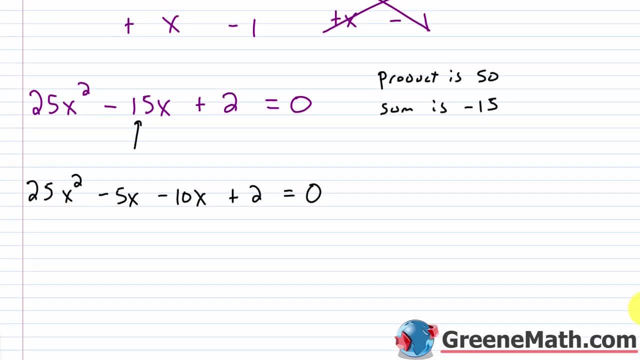 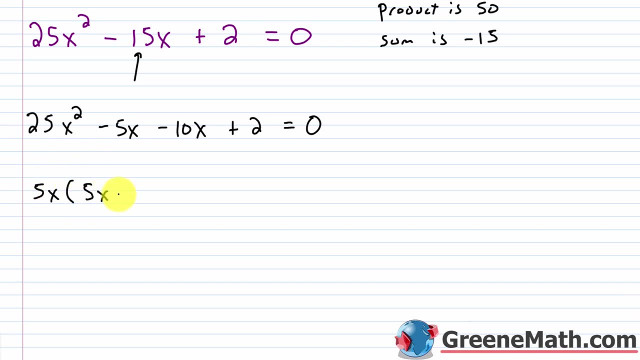 So now that I have a four term Polynomial, I'm going to just factor using grouping. So from the first group I could pull out a five x. That would leave me with five x minus one. from the second group, Because I want to match the signs, I'm going to pull out a negative. 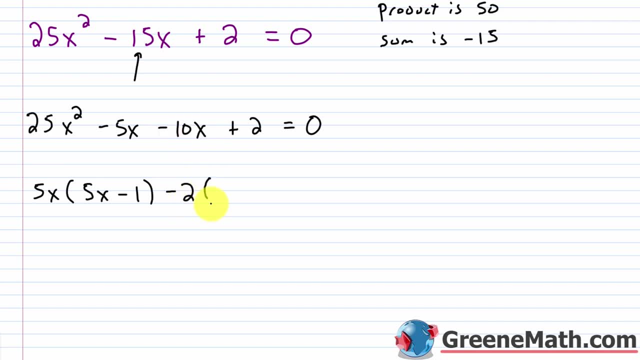 and I'm going to be pulling out a negative two. So minus two here, and then we'll have five x minus one. So we see we have a common binomial factor of this five x minus one, and we're going to pull out a negative two. 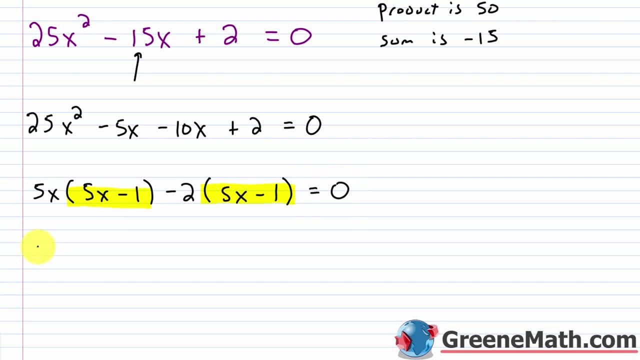 So I'm going to pull that out. So I'll set this equal to zero. We'll pull that out. We'll have five x minus one, that quantity multiplied by five x minus two, That quantity is equals zero. All right, So again, I have two factors here. 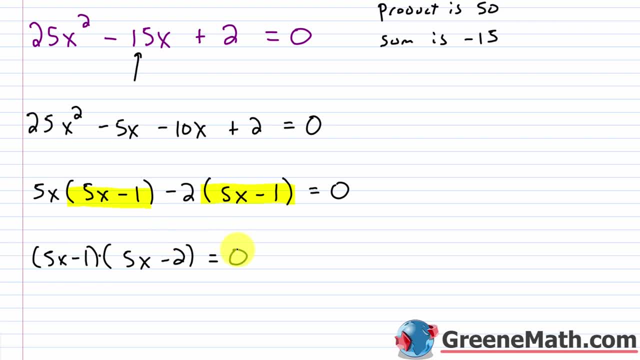 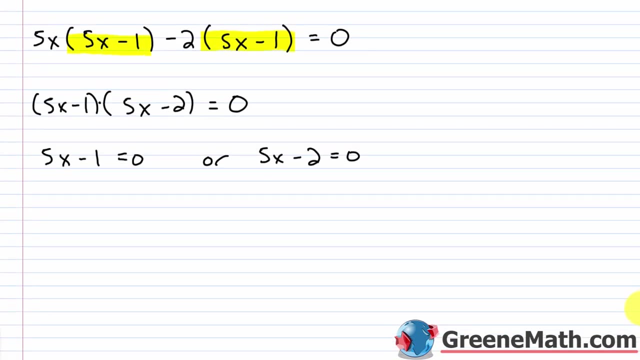 This is multiplication, So this times this gives me zero. So it must be true that five x minus one equals zero, or five x minus two equals zero. So we just need to solve each equation So we can get our solution here. So what we want to do, let's just add one to both sides. 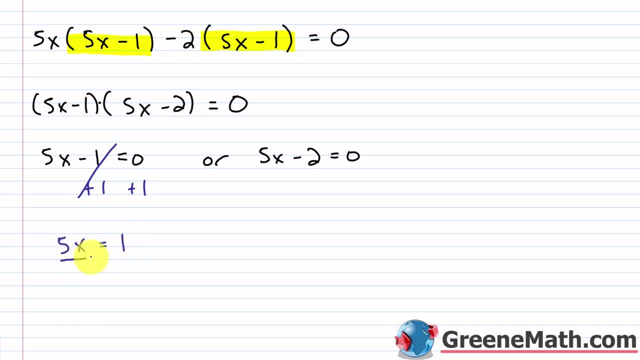 That'll cancel. You'll have five. x is equal to one. Divide both sides by five and you'll get x is equal to one. fifth Over here. if I add two to both sides of the equation, that'll cancel. You'll have five. x is equal to two. 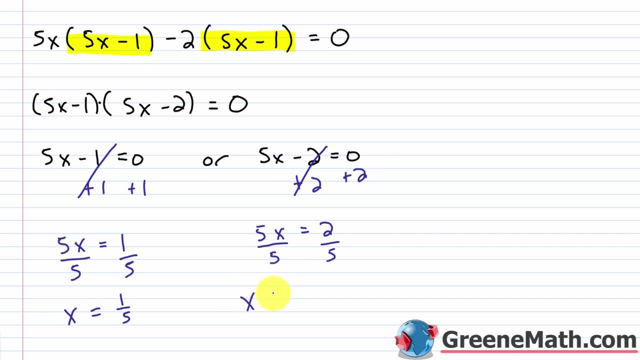 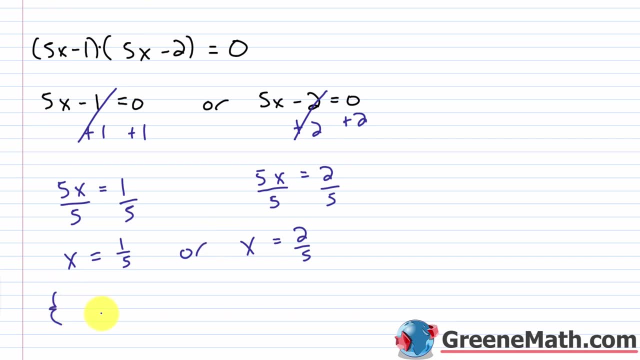 Divide both sides by five and you'll get x is equal to two fifths. So in solution set notation we'll say: inside of curly braces we have one fifth, comma two fifths. So those are our two solutions: x equals one fifth or x equals two fifths. 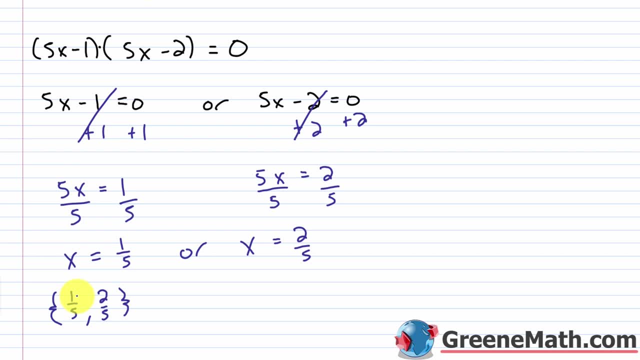 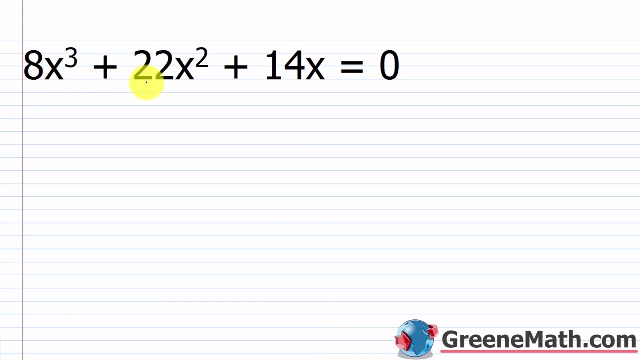 Again. you can pause the video, check each solution and verify that we got the correct answer. All right, For the last one we're going to look at. we have eight x cubed plus 22 x squared, plus 14 x equals zero. 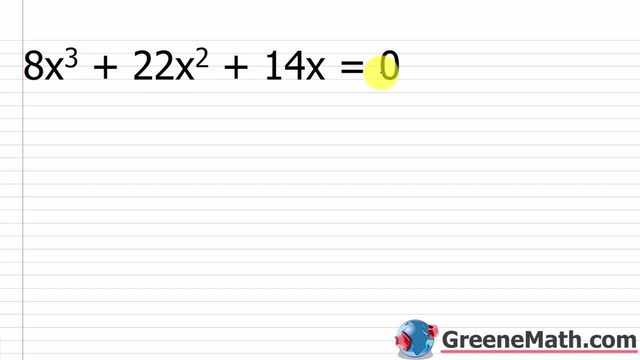 So you might jump out and say, well, that's not true, That's not true, That's not true. Whoa, that's not a quadratic equation. When we can factor something like we will be able to: here, you're going to end up being able to get the solution that way, versus using some other method. 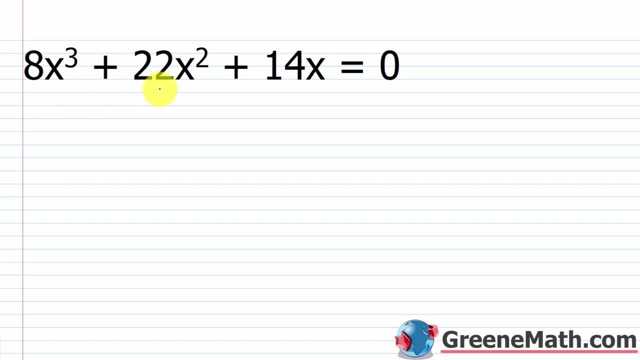 So, for eight x cubed plus 22 x squared plus 14 x equals zero. on the left side it's already in standard form. The first thing you should notice is that there's a common factor of x and there's also a common factor of two. 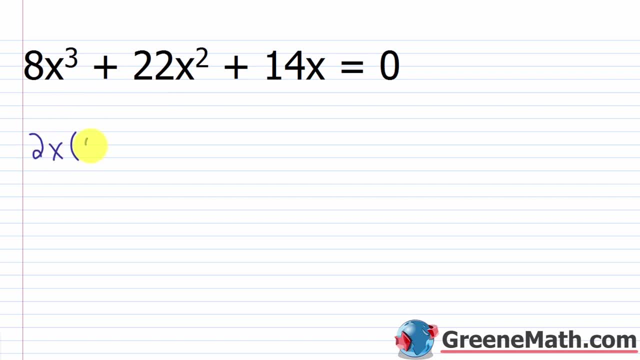 So I could pull out a two x and what would be left is four x squared plus 11 x plus seven. This is equal to zero. Now, inside the parentheses, we have a quadratic equation. So again, that's something that's familiar to us. 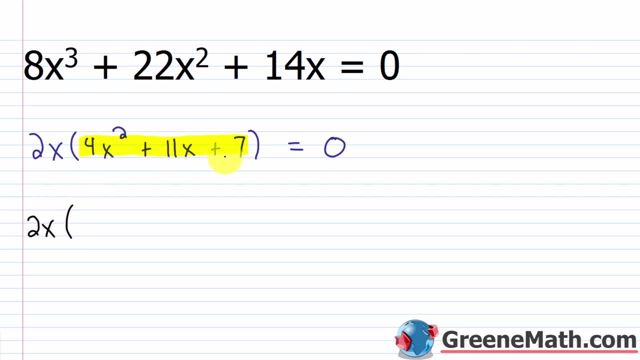 So we have our two x. that just stays out in front and I want to just factor the inside. So if I think about two integers, whose product would be what? Four times seven is 28.. So we think about a product of 28.. 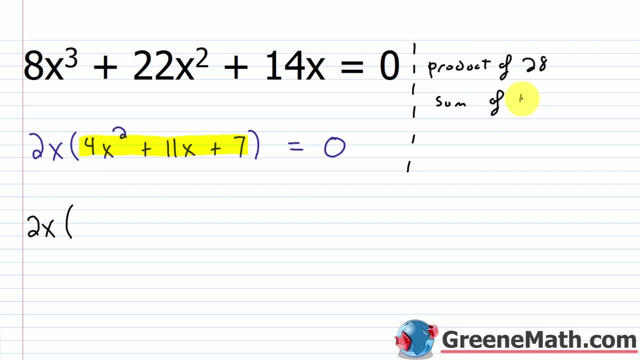 And a sum of 11.. Well, four and seven give me that criteria. Four plus seven is 11.. Four times seven is 28.. So again use that to rewrite that middle term there. So I would have four x squared, then plus. we'll do four x, then plus seven x. 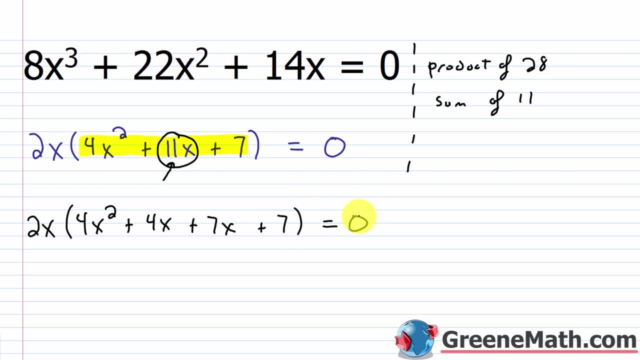 then plus seven, and this equals zero. All right, so I'm going to have my two x here. From the first group, I can pull out a four x. Then inside I would have x plus one. From the second group, I can pull out a seven. 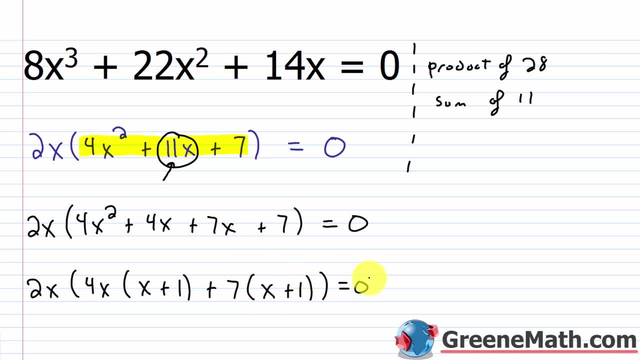 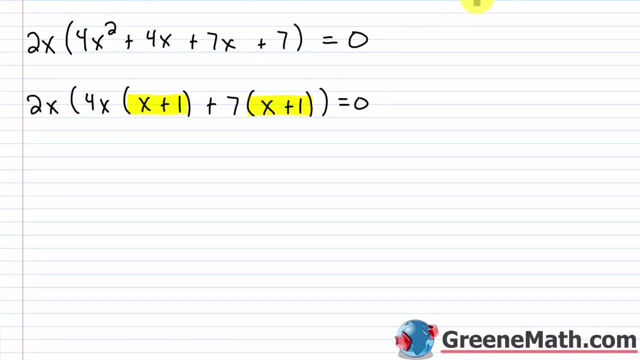 Then inside I'd have x plus one. So you have your common binomial factor. Let me just kind of scroll down a little bit. You have your common binomial factor of x plus one, that quantity, And we can factor that out. 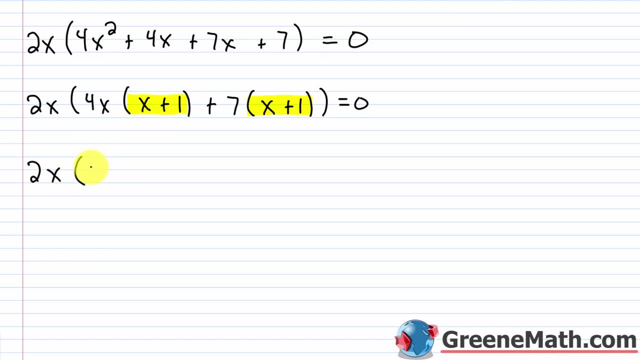 So I'm going to have my two x out in front. I'll have that quantity x plus one, And then what's left? We'll have four x plus seven. Now this equals zero. So now I have three factors here with a variable. 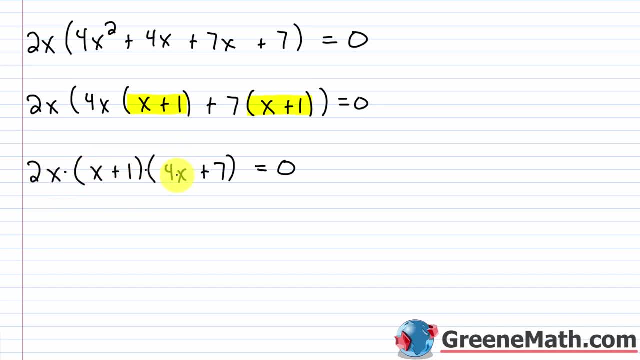 Two x is multiplied by the quantity x plus one, which is multiplied by the quantity four x plus seven. So I've got to set each one equal to zero Again. let me label this so it's crystal clear: This is a factor. 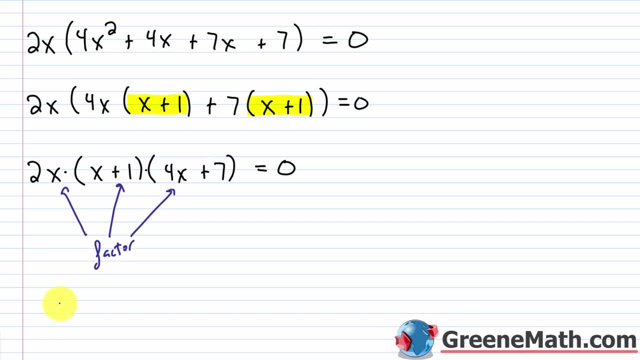 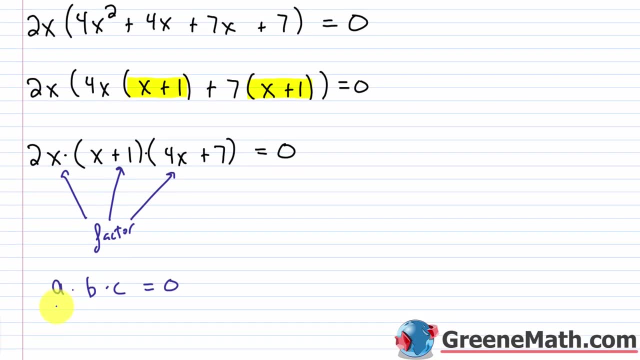 This is a factor. And this is a factor, Just like if I had a times b times c equals zero. it's got to be true that a equals zero or b equals zero or c equals zero, or it can actually be a factor. 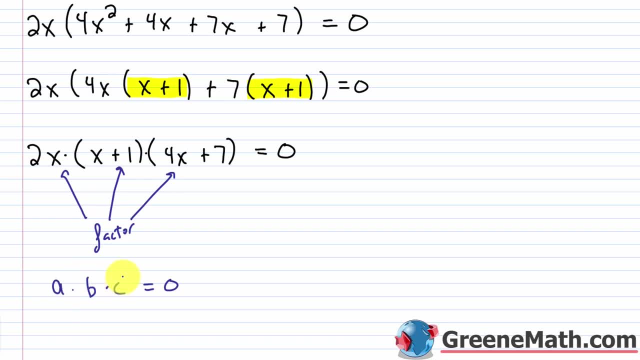 In this case because we have three of them. any two of them equals zero and the other one doesn't, or all three of them equals zero. So lots of possibilities, But the point is here that each one of these has to be set equal to zero. 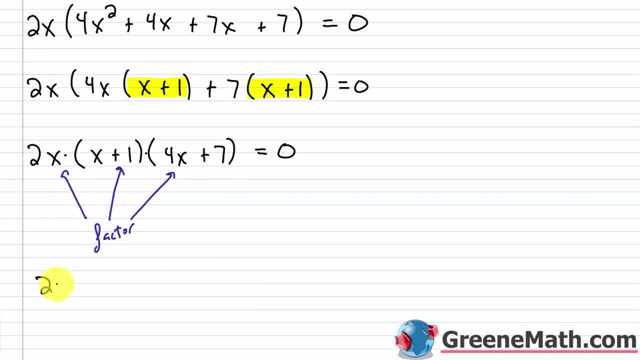 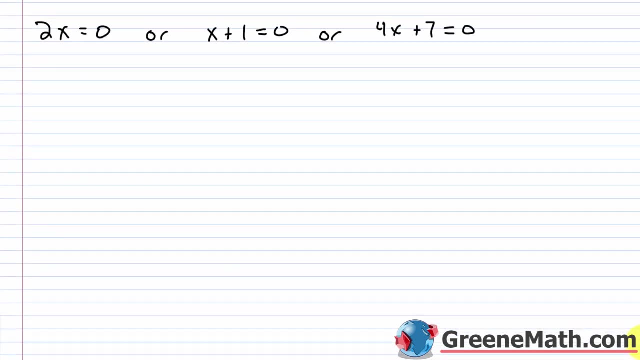 because it's a possible solution for us. So we would say two x is equal to zero, or x plus one is equal to zero, or four x plus seven is equal to zero. So let's solve these three equations All right. Two x equals zero is very simple. 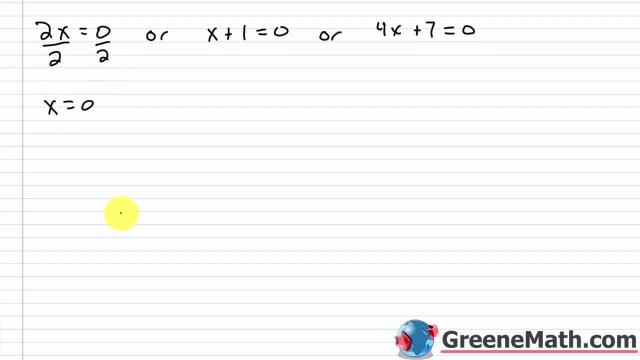 You divide both sides by two, You get x equals zero. Then for this one: x plus one equals zero. We subtract one away from each side, We get x is equal to negative one. Then for four: x plus seven equals zero. we subtract seven away from each side. 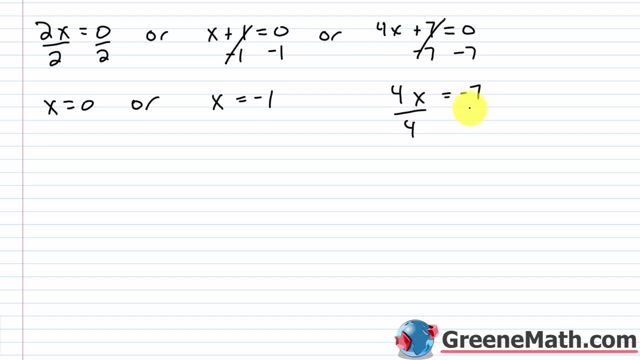 We get four, x is equal to negative seven. We divide both sides by four, We get x is equal to negative seven fourths. So I'll put my, or kind of like that. So we get x equals zero Or x equals negative one. 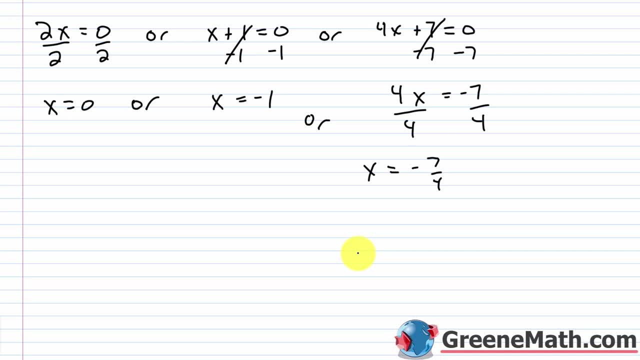 Or x equals negative seven fourths. So in a solution set notation we put negative seven fourths comma negative one comma zero. So those are your three solutions. Now again, if you want to check this, go back to the original equation. 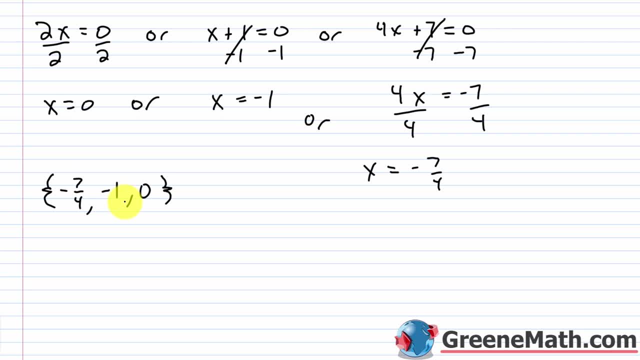 You're going to plug in a negative seven fourths for x and plug in a negative one for x and plug in a zero for x. In each case, you're going to verify that the left and the right side are equal. All right. 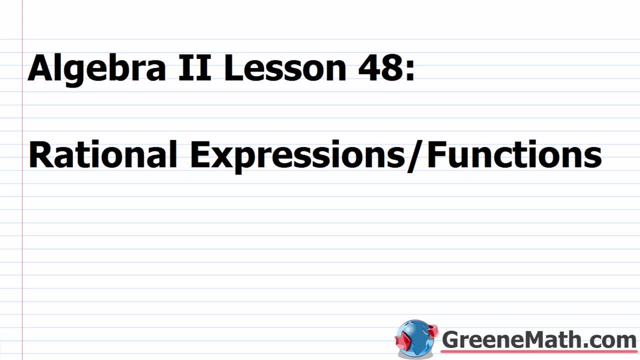 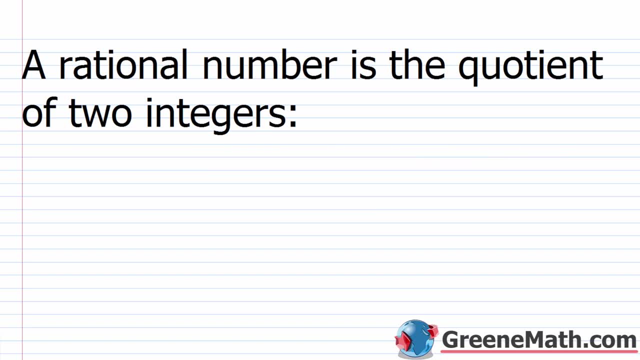 Hello and welcome to Algebra 2, Lesson 48.. In this video we're going to learn about rational expressions and rational functions. So the majority of you worked with rational expressions back in Algebra 1.. At this point you just need to know that working with a rational expression 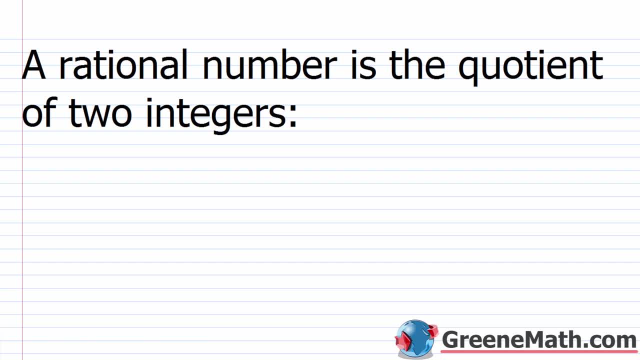 is in many ways identical to working with fractions, So let's just start out by talking about fractions a little bit. So we should know at this point that a rational number is the quotient of two integers. So some examples, Some examples of a rational number. 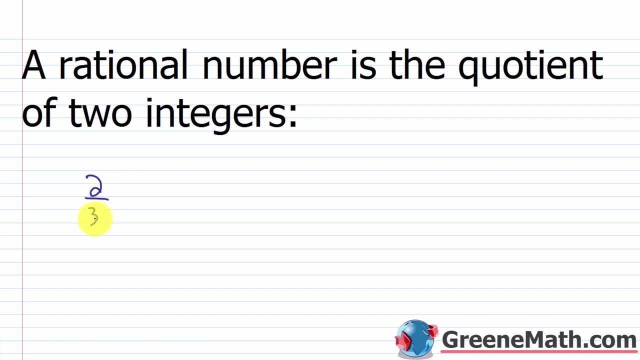 Something like two thirds. So I have an integer two over an integer three. Something like five sevenths, Integer five over an integer seven. Something like negative two. elevenths, An integer of negative two over an integer of eleven. So very easy to define a rational number. 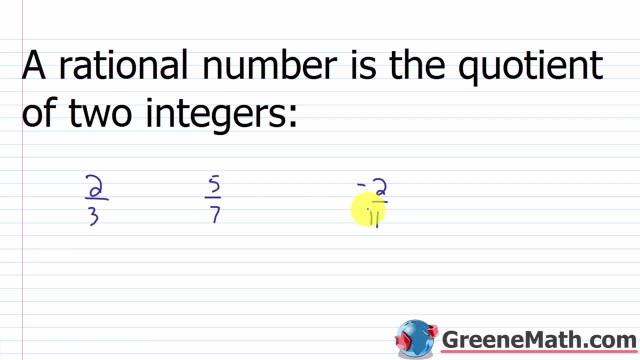 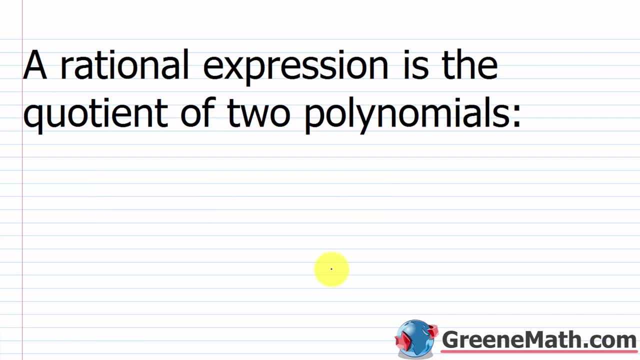 The one restriction is that one: We cannot have the integer zero in the denominator, because division by zero is considered undefined. So just like we have rational numbers which are the quotient of two integers, we have rational expressions, So a rational expression is the quotient of two polynomials. 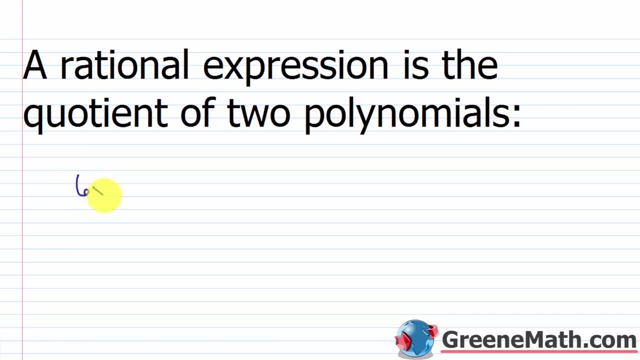 So just to give you two examples, let's say it's something like six x squared minus five, And this was over x cubed. This is a polynomial. It's a binomial in the numerator. This is a polynomial, It's a monomial in the denominator. 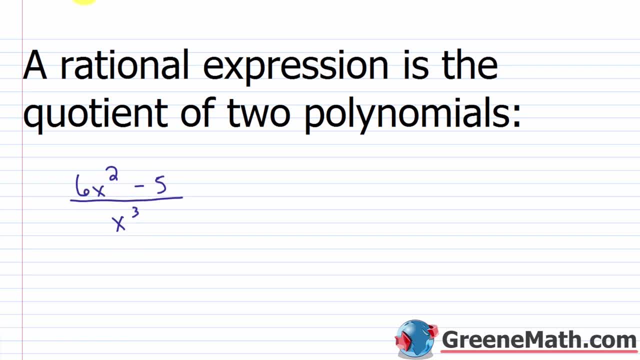 So this is a rational expression. Or as another example, let's say you had something like three x to the seventh power, minus five x cubed, plus two x minus one over. let's say you just had something like four x to the fifth power. 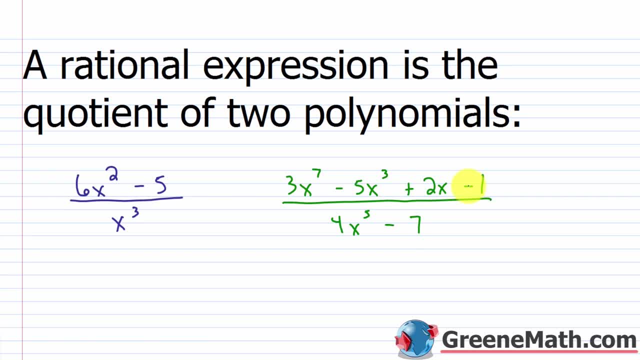 minus seven. So you've got a polynomial in the numerator over a polynomial in the denominator. So this is considered a rational expression. Now in your textbook you're probably going to see something that looks a little bit confusing. They will start out by saying that a rational expression is what? 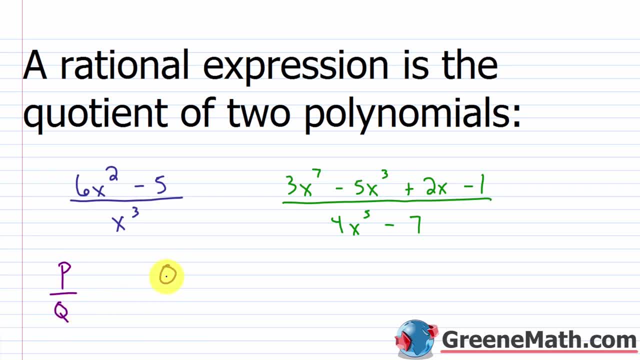 It's p over q, where q does not equal zero, And I want to talk about this for a minute because we're going to go into a section where we're talking about this denominator not being allowed to be equal to zero. So p is a polynomial and q is a polynomial. 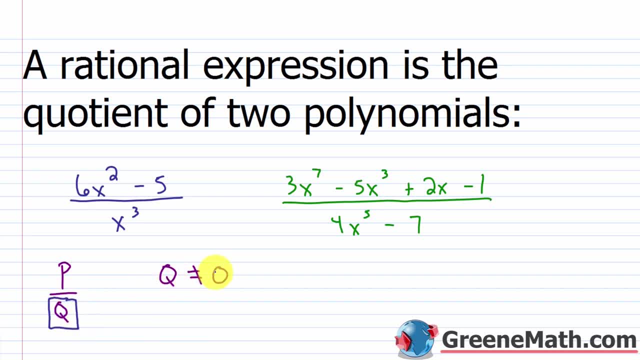 But q lies in the denominator And we say q cannot be equal to zero because, again, we can never divide by zero, Because division by zero is undefined. So, specifically, what we're saying is that if we have a rational expression, generally speaking, we have variables in our denominator. 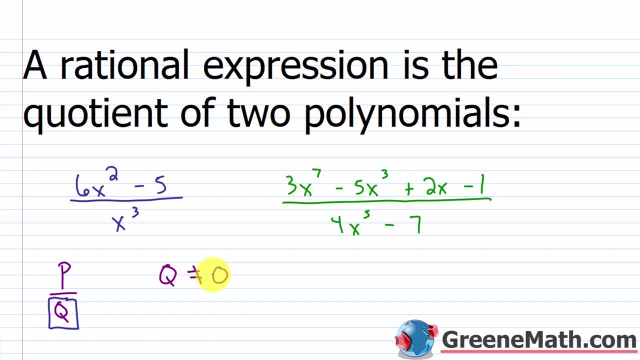 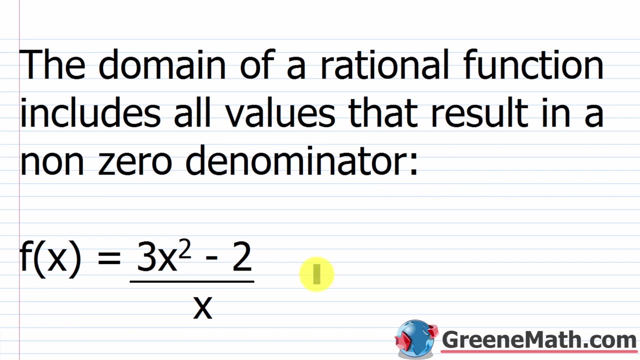 Sometimes you won't, but in most cases you will. So we want to say that that variable cannot be equal to any value that results in the denominator becoming zero. So I want to start out by just talking about finding the domain of a rational expression. 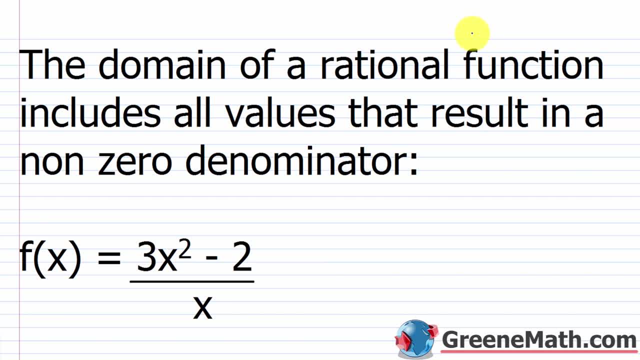 So I want you to recall that the domain- we talked about this when we talked about functions- is the set of allowable x values. So the domain or the set of allowable x values of a rational function includes all values that result in a non-zero denominator. 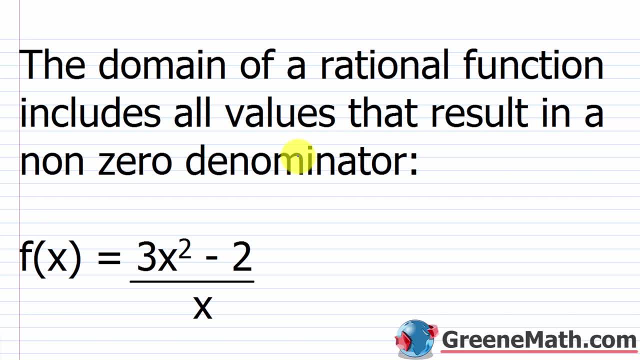 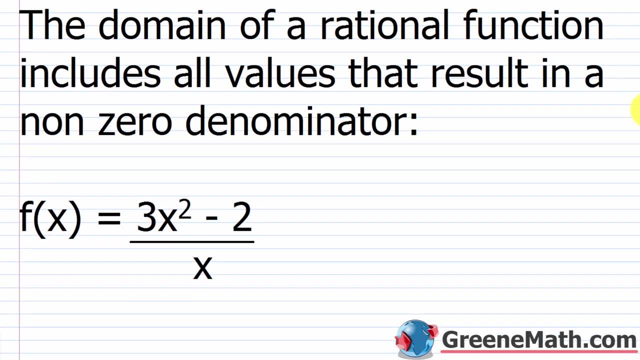 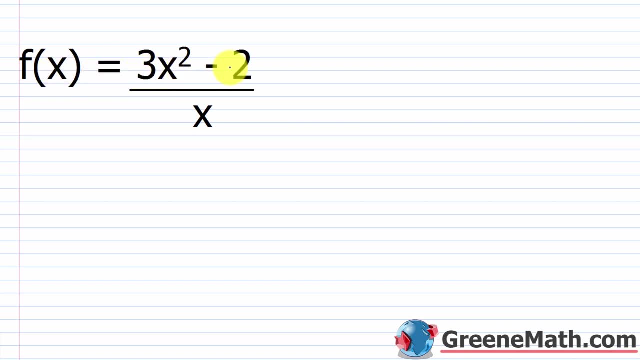 So what's allowable here for x is anything that does not result in the denominator being zero. Now for the first problem we're going to look at, and we're just going to find the domain. it's very, very simple. If I look at, f of x is equal to 3x squared minus 2 over x, and I say: well, what's the domain? 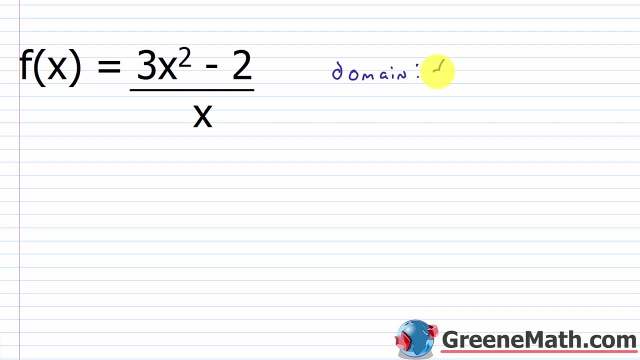 What is the domain? All you need to think about if you get this problem is look at the denominator and say: what can I not plug in for that variable Because, again, I don't want the result to be zero. Well, it's very straightforward here. 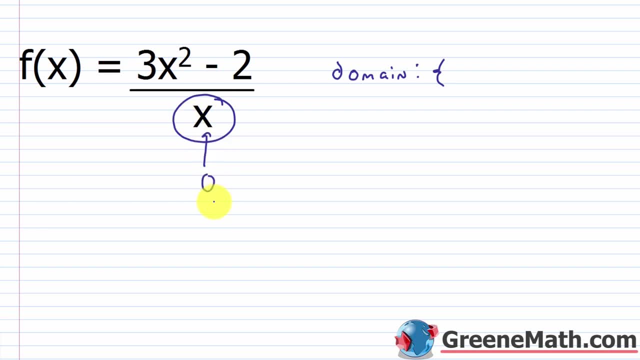 I just cannot plug in a zero. If I plugged in a zero for x, I'd be dividing by zero, which is not allowed. So the domain would be the set of all x values, such that x does not equal zero. Okay, And again, I put this in set builder notation. 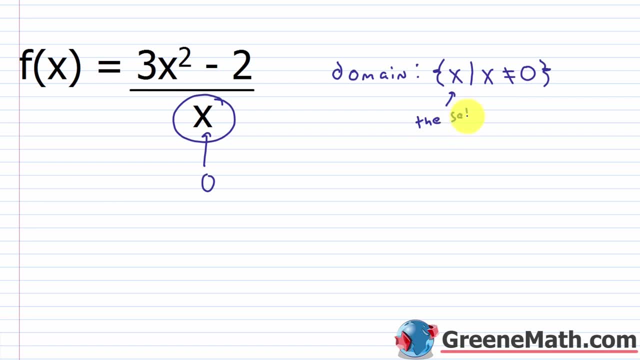 So let me just write this out: This is the set of all x. We have this such that that real number you choose, which is x, it can't be equal to zero, So I can choose any other value that I'd like. 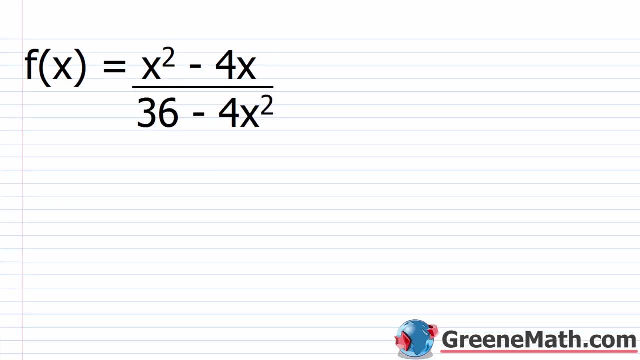 All right, So that's your domain for this one. For this one it's going to be a little bit more complicated. We have f of x is equal to. we have x squared minus 4x over 36 minus 4x squared. 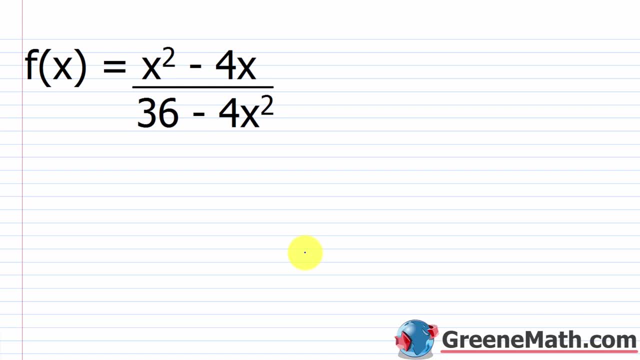 What I want to think about is a value- or it could be values- for the variable x. that would result in this whole thing becoming zero. So, in order to do that, what do I need to do? I need to set up a value. 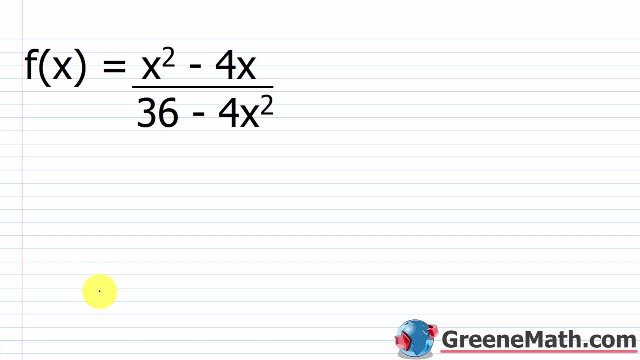 I need to set up and solve an equation. What I need to do is say: well, 36 minus 4x squared cannot be equal to zero, or I could put equal zero, And then if I find a value or values that make this equation true, then they have to. 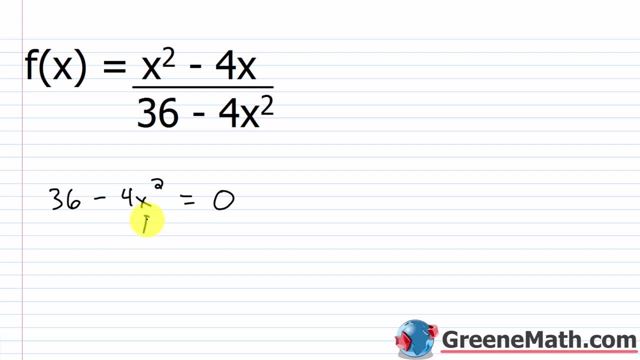 be excluded, because if I plug in for x there and I evaluate, I'll end up with zero, And I don't want that for my denominator. So how could we solve something like that? I know we talked about the quadratic formula in Algebra 1,, but we haven't really got to. 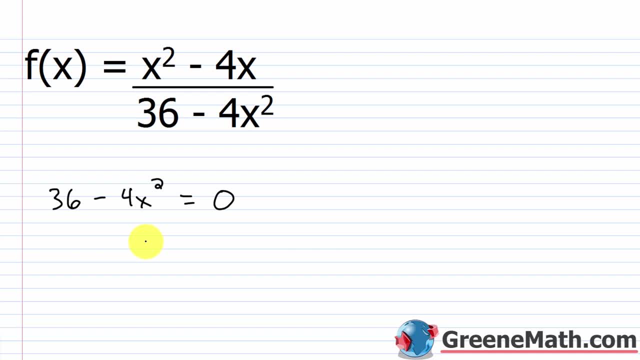 it in Algebra 2 yet, so I'm going to stick with things that we can solve via factoring. This is the difference of two squares. This is 6 squared minus 2x squared. We could factor this into 6 plus 2x that quantity times 6 minus 2x that quantity. 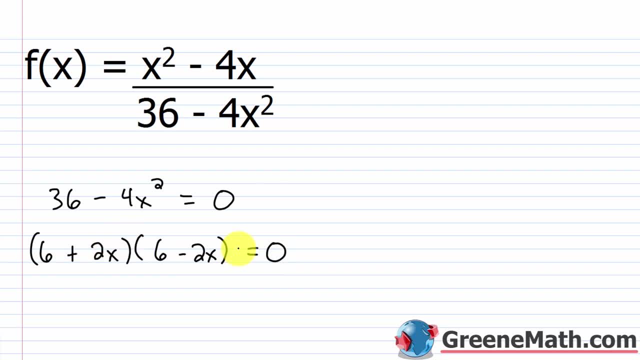 We set this equal to zero, We can use our zero product property. this factor here, 6 plus 2x would be equal to 0. And then, OR we'd have: 6 minus 2x is equal to 0.. 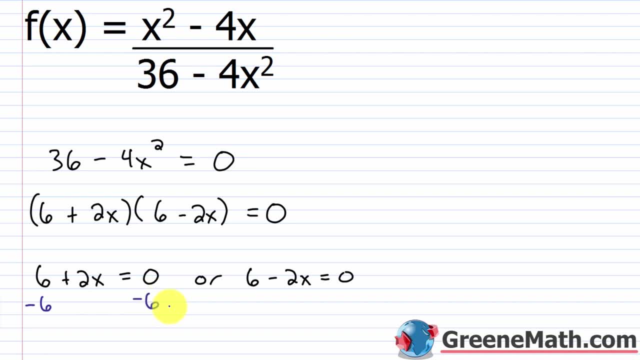 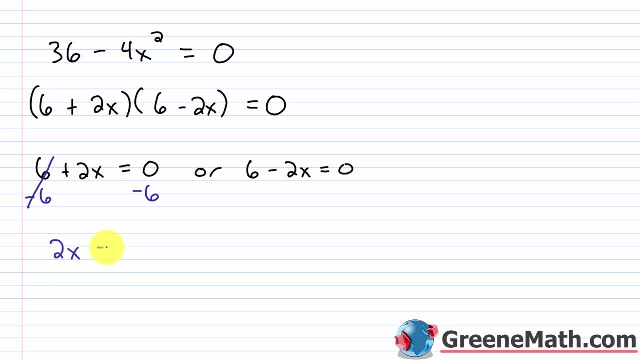 Let's go ahead and subtract 6 away from each side of the equation, So this would cancel. Let me scroll down and get some room going here, And what we're going to have is 2x is equal to negative 6. Divide both sides by 2, and we'll get that x is equal to negative 3.. Over here, let's subtract. 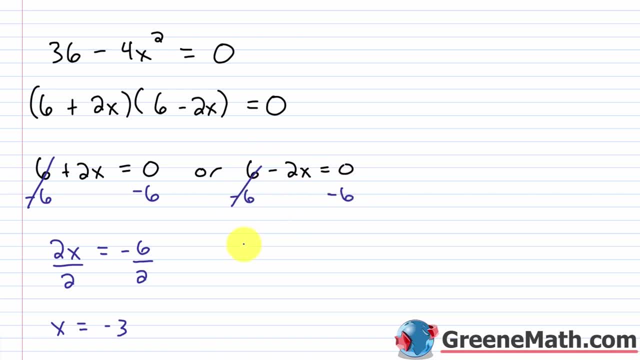 6 away from each side of the equation. This will cancel. We'll have negative 2x is equal to negative 6.. What we'll do is we'll divide both sides of the equation by negative 2, and we'll have that x is. 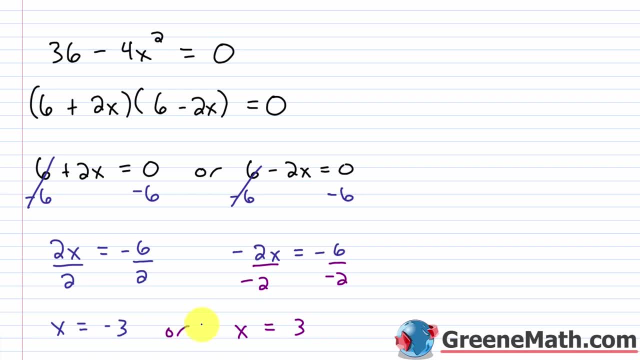 equal to 3.. Let me put my OR there, So x equals negative 3, or x equals 3.. So you have to remember what we're doing here. Let me erase everything, So let me just put this off to the side, as like. 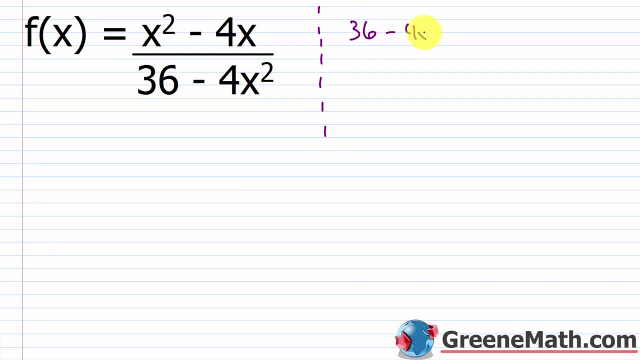 a little note. We solved 36 minus 4x Squared equals 0.. And the solution set contained two elements: negative 3 and 3.. So what that's telling me is that if I plug in a 3 or a negative 3 in for x there. so if I plugged, 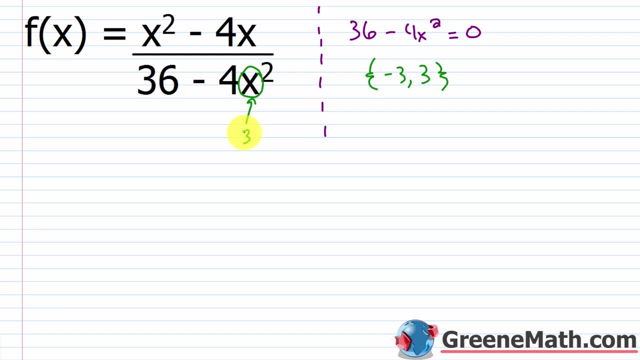 in a 3, let's just start with that- you would get a 0 as your denominator, and that's not allowed. So you would have 36 minus 4 times 3, squared is 9.. So 4 times 9 is 36.. So you get 36 minus 36,. 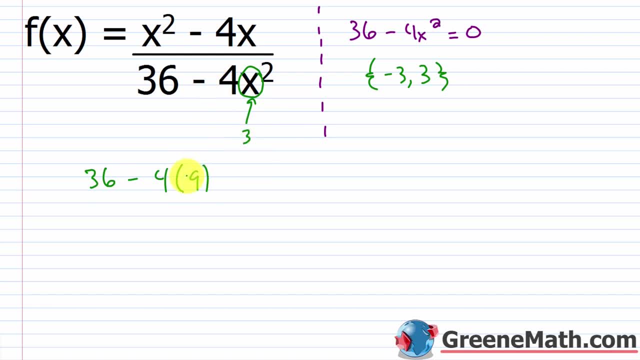 which is 0.. It would be the same thing if I plugged in a negative 3,, because you'd have negative 3 squared, which is positive 9.. Again, you get 36 minus 36,, which would be 0.. 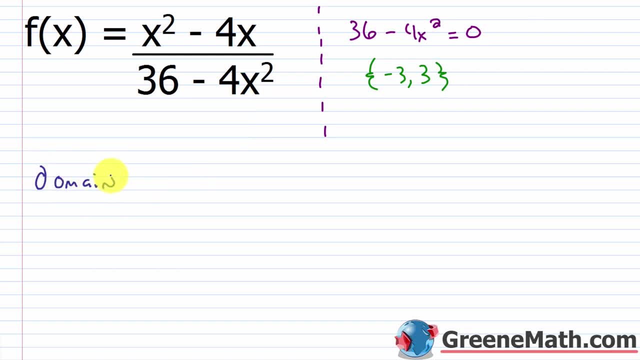 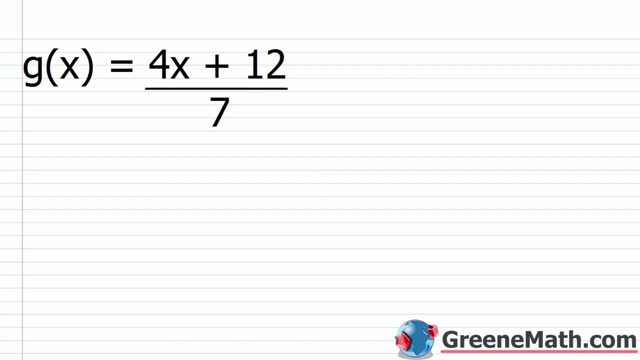 So then, the domain here, the domain is the set of all x values, such that x does not equal negative 3 or 3.. So negative, 3 or 3.. So let's take a look at one last one. So we have, g of x is equal to 4x plus 12,. 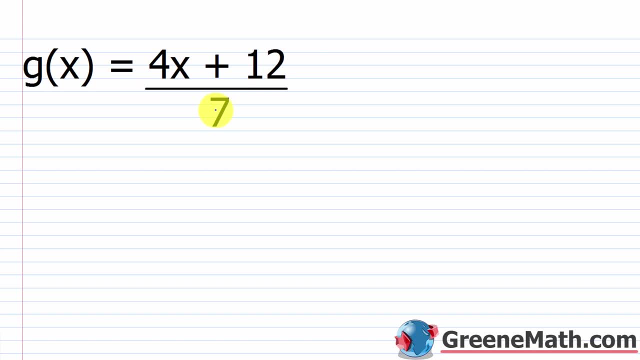 over 7.. So in this case, is there going to be any restriction on the domain? No, there's not. I don't have a variable in the denominator, so I'm basically good to go. So for something like this, we would say: the domain. the domain is the set of all real numbers. Okay, pretty simple. 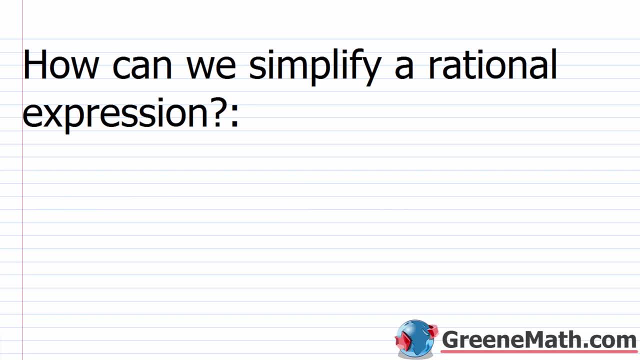 overall All right. so now let's talk about kind of the next topic that comes up when you talk about rational expressions for the first time. So let's talk about the next topic that comes up when you talk about rational expressions for the first time: How can we simplify a rational expression? 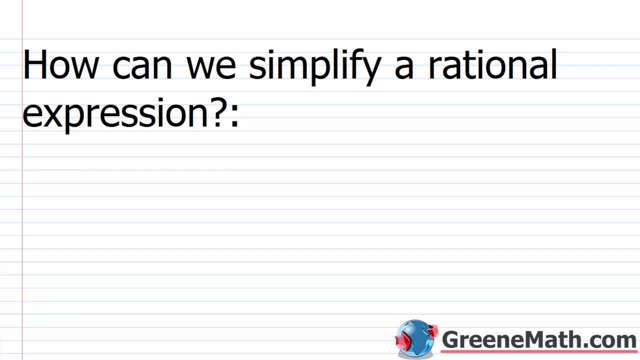 Well, it goes back to simplifying a fraction. So if I have something like 2 over 4, we know that we can cancel the greatest common factor between numerator and denominator. Now, a lot of us at this point we know that 2 and 4 share a common factor of 2.. So you can say, okay, 2 divided by 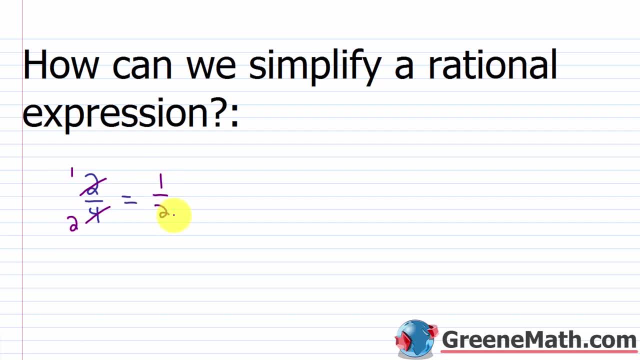 2 is 1,, 4 divided by 2 is 2.. So you end up with one half, like that. But if you didn't know, that, off the top of your head, which you're not going to know this and you're not going to know this, 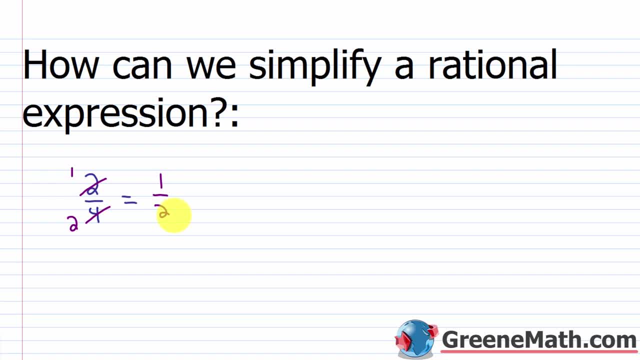 in the case of a lot of rational expressions, you would factor it right, So you would say: okay, well, 2 is a prime number. So really the best I could do is say 2 times 1, and 4 is 2 times. 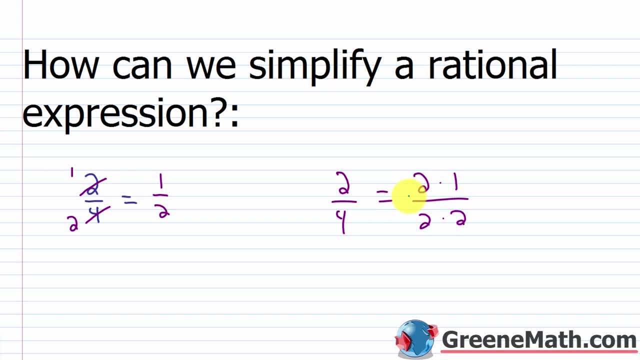 2.. So then, when you look at it like this, it's obvious that you cancel a common factor of 2 between numerator and denominator and you're left with one half. Okay. so this is basically the process that we're going to use to simplify a rational expression. Well, let's go ahead and 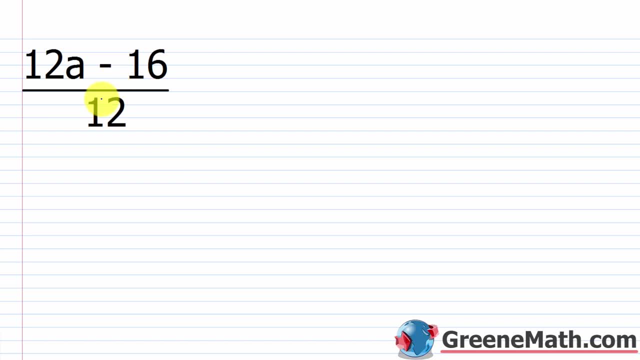 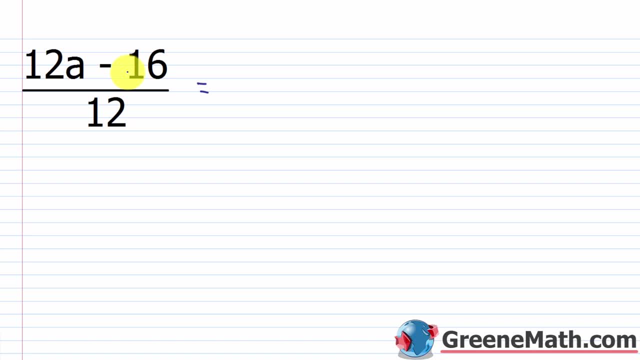 numerator and I want to factor out the greatest common factor. So between 12 and 16, it's going to be 4.. So if I pull a 4 out, I'll have 4 times the quantity. Inside of parentheses I'll have 3a. 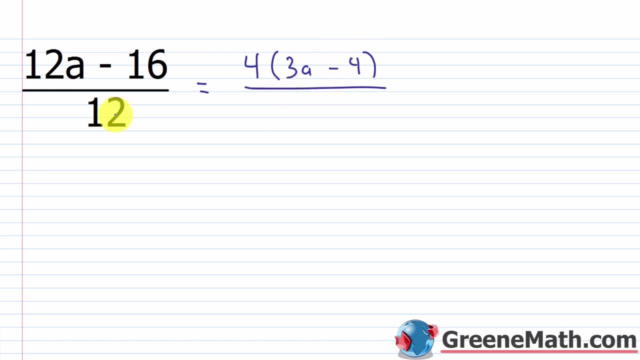 minus 4.. Then down here I have 12, which is divisible by 4.. So I could write this as 4 times 3.. Now one thing I want you to realize is that this is multiple times 4.. So if I pull a 4 out, I'll have 4 times the quantity Inside of parentheses. 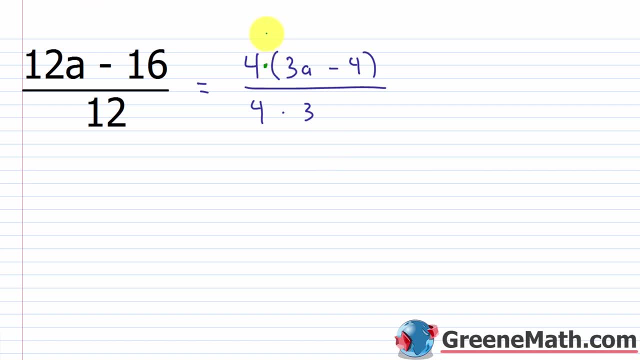 this is multiplication, right here, This is multiplication. So this 4 is a factor And this quantity, 3a- OK, 3a minus 4 is a factor. OK, 4 is multiplying that entire thing, So we are able to. 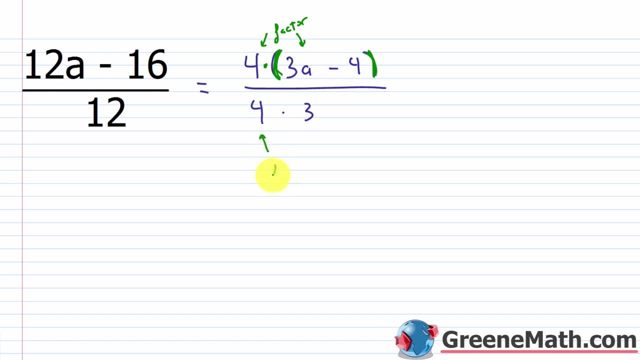 cancel common factors. This is a factor, And this is a factor. So between the numerator and denominator they share a common factor of 4.. So that can be canceled. So we have 12.5.. So we have 3a minus 4.. So what's left? now You have the quantity 3a minus 4.. I don't need the parentheses. 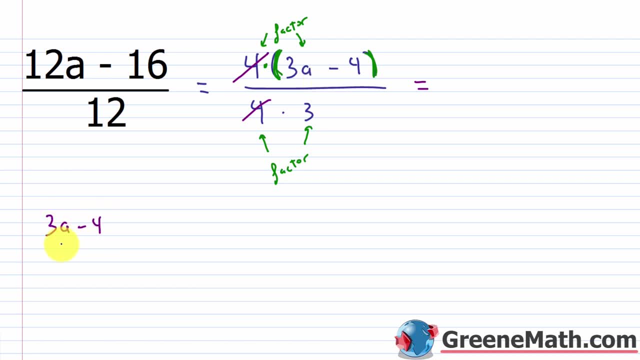 anymore. I can just get rid of them. So 3a minus 4. And then over just 3.. Now here's where students make a gigantic mistake. We just talked about common factors, And I know it's confusing because 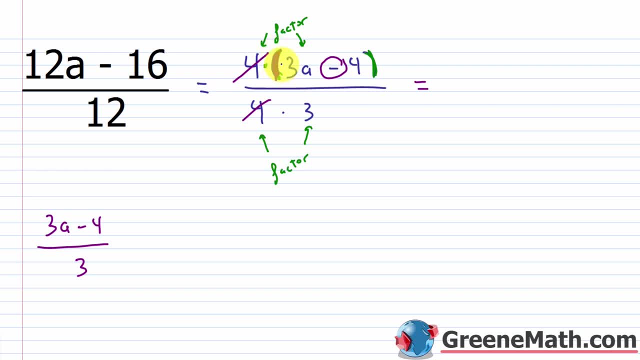 there's a minus sign in here, But it's this entire thing that's being multiplied by 4 there, So those two are factors. Here I just have 3a minus 4.. And then over just 3.. Now here's where students. 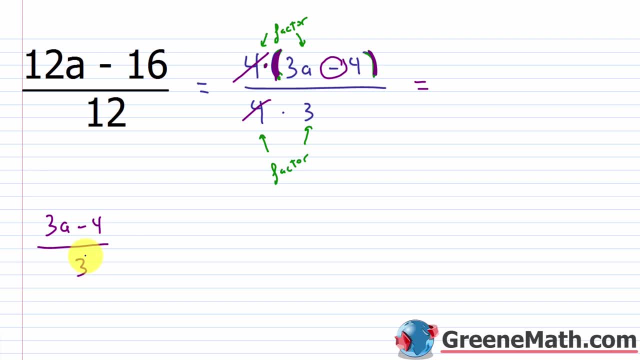 make a gigantic mistake. We just have 3a minus 4 over 3.. There's no common factor between the numerator and denominator other than 1.. All right, I could do this. if I wanted to. I could put this in parentheses and say times 1.. I could put this times 1.. And then, if you wanted to cancel 1 with, 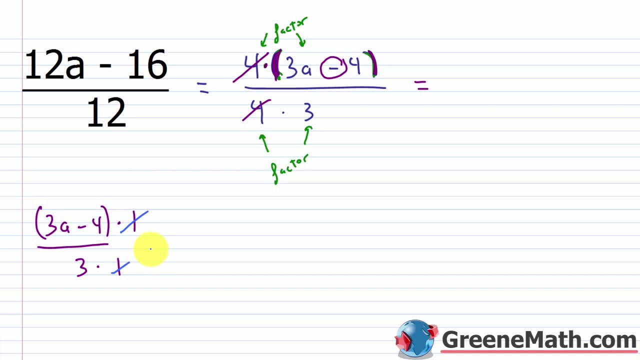 1,, it wouldn't do anything right. It's still just equal to 1.. But that's an example of something you could actually do. But because I don't have any common factors, I can't just go through and do this. I can't say: OK, well, I've got a 3a minus 4.. I can't just go through and do this. I can't. 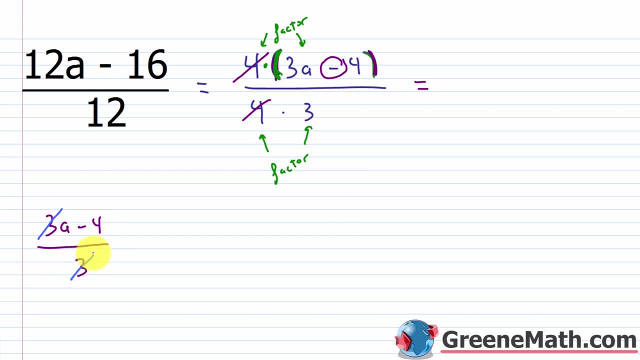 say: OK, well, I've got a 3 here and a 3 here. That's a very common mistake that you're going to see. Let me just label this as a common mistake, And you see it in Algebra 1.. You definitely still. 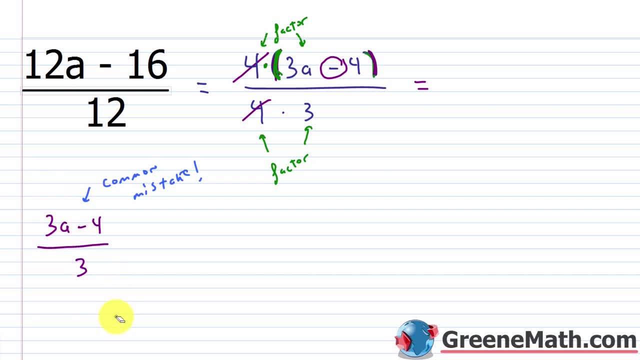 see it in Algebra 2.. It's something you have to realize that is illegal. Your answer here, your simplified result, is 3a minus 4 over 3, right, Nothing else you can do. All right, let's take a look at the next problem. So we have x squared minus 9x plus 8.. 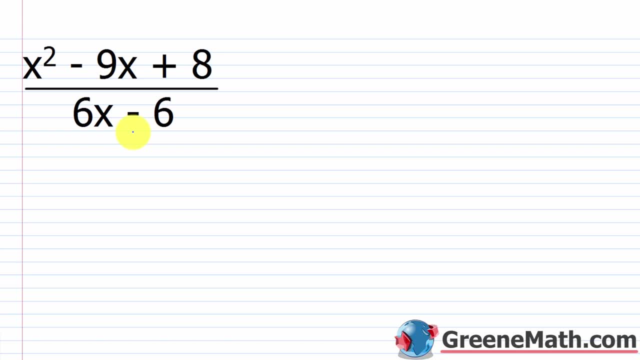 Over 6x minus 6.. What you want to do here is you want to factor the numerator and denominator and see which you can cancel. So in the numerator we have a trinomial, So we're going to factor that as the product of two binomials. So it's an easy scenario I have. 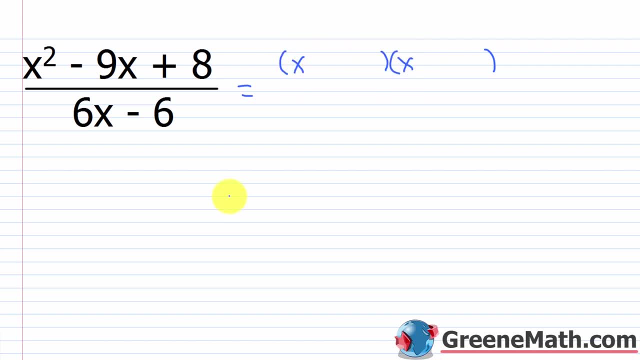 x squared. So I'm going to put x here and x here And then just find two integers whose sum is negative 9 and whose product is positive 8. Well, that would be negative 8 and negative 1. Then we'll put in the denominator and the denominator, And then we'll put in the denominator. 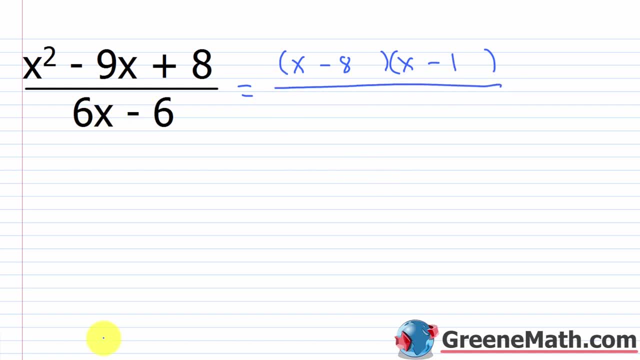 and the denominator, And then we'll put this over. We have 6x minus 6.. I could factor out a 6 from that, And I'd be left with x minus 1 inside a parentheses. So again, this is multiplication. 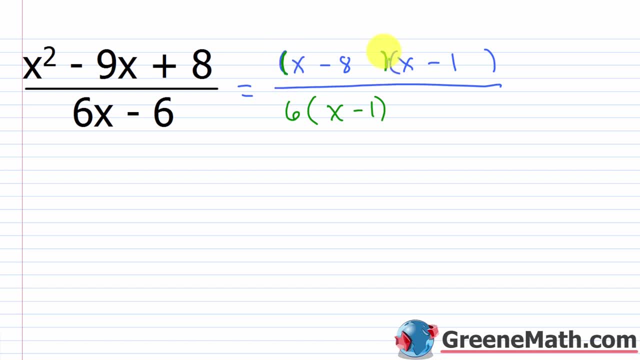 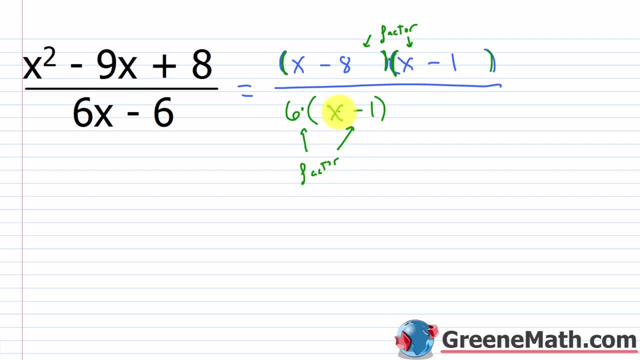 So this is a factor. And then so is this, This quantity x minus 1.. So do I have a common factor between the numerator and denominator? Yeah, I have the quantity x minus 1.. This can be canceled with this. They're common factors. So what I'm left with is x minus 8 over 6.. Now 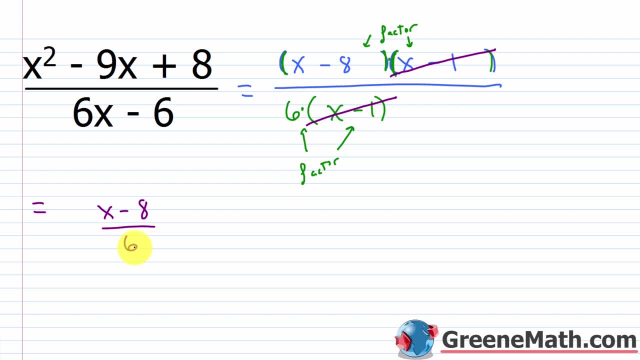 this is something that you really need to understand. You might be given a second task on a problem like this And they might say: state the restricted values as well as, to simplify, Is this right here: this x squared minus 9x plus 8 over 6x minus 6, the same as x minus 8 over 6?. 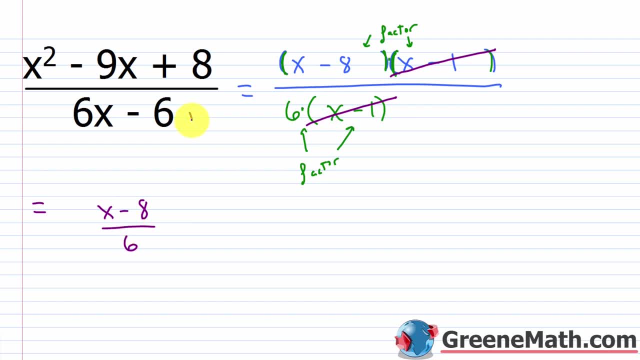 Not technically, Because, if I think about this right here, x cannot be equal to 1. Because if I plug the 1 in there 6 times 1 is 6. And then 6 minus 6 would be 0. So with this original 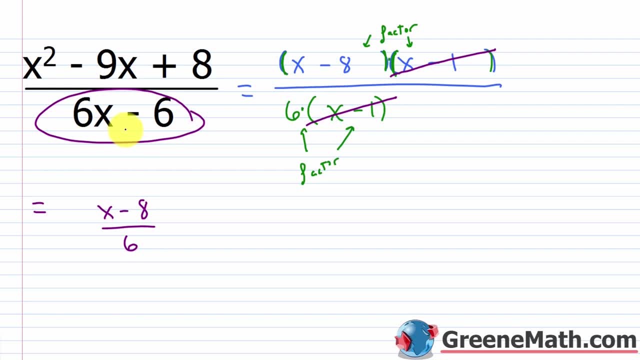 rational expression, we're going to have a problem like this. We're going to have a problem like this: We have a restriction where x cannot be 1.. In this simplified version right here, x can be whatever you want, because there's no variable in the denominator. 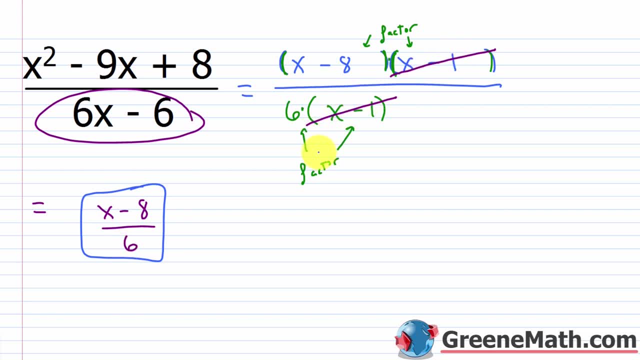 By canceling a common factor, we have lost some information. We have lost some information. So if you're going to be given a task like this, you want to find the restricted values before you do any simplification. So we would say that in this case, x cannot be equal to 1.. 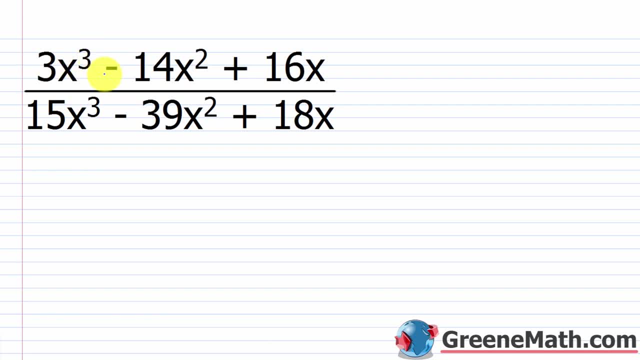 Now let's take a look at the next example. So we have 3 x cubed minus 14 x squared plus 16 x, And this is over 15 x cubed minus 39 x squared plus 18 x. So we want to simplify here. 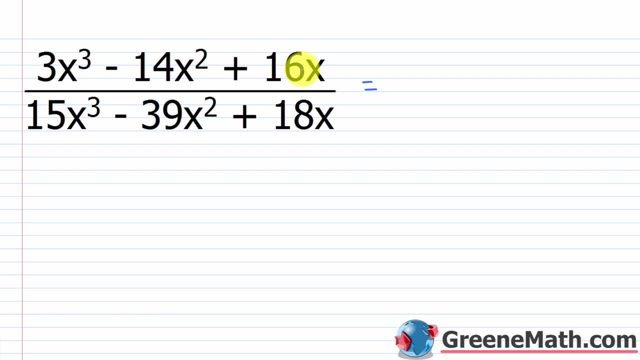 So in the numerator, what can I do to factor? Well, you would notice that everything has an x, So I could pull that out to start And I would have 3 x squared minus 14, x plus 16. And this is over. 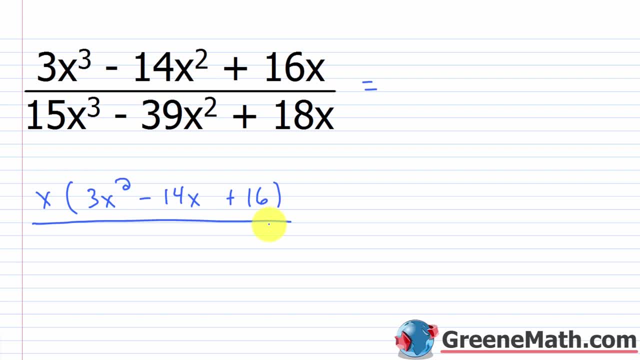 denominator. everything has a 3, that's common, and everything also has an x. So let's pull out a 3x and I'd have 5x squared minus 13x plus 6.. Now what I'm going to do is factor this and this: 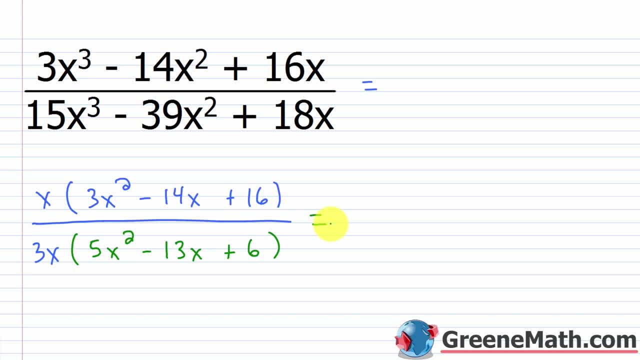 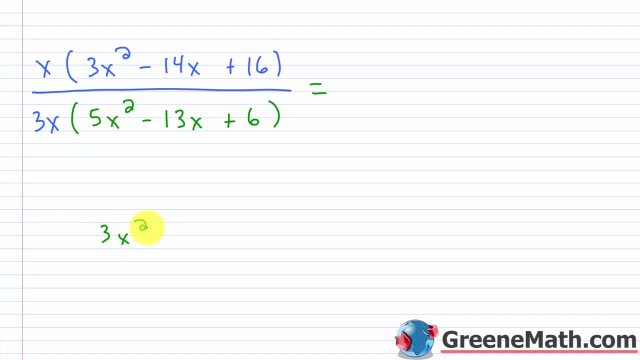 each of those into the product of two binomials. So in the numerator we kind of scroll down, get some room going. I have 3x squared minus 14x plus 16.. So I'm going to factor this using factoring by grouping. If I think about it, I want two integers whose product is 3 times 16, which is 48. 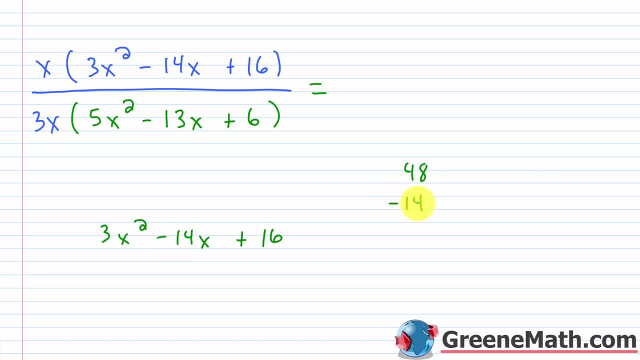 and whose sum is negative 14.. So I know I need a negative and another negative. So think about some factors of 48.. We've got 1 and 48,, 2 and 24,, 3 and 7, and 8. So I'm going to factor this using factoring by grouping. So I'm going to factor this. 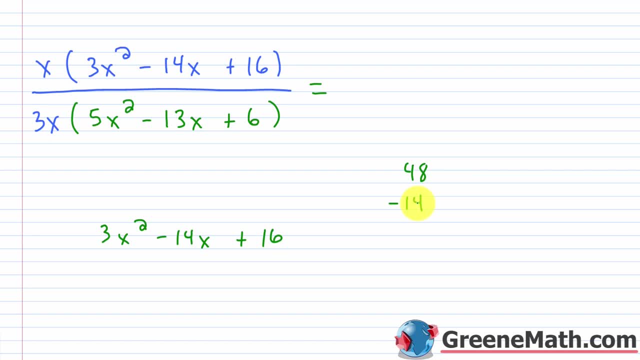 16,, 4 and 12, and then 6 and 8.. If I had negative 6 and negative 8, that would work. So I'm going to rewrite this middle term here. I'm going to say: this is 3x squared minus 6x. 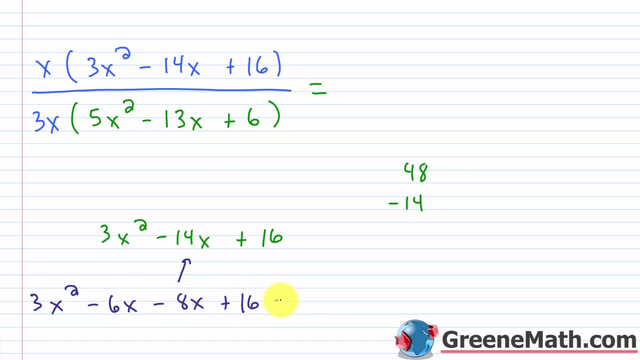 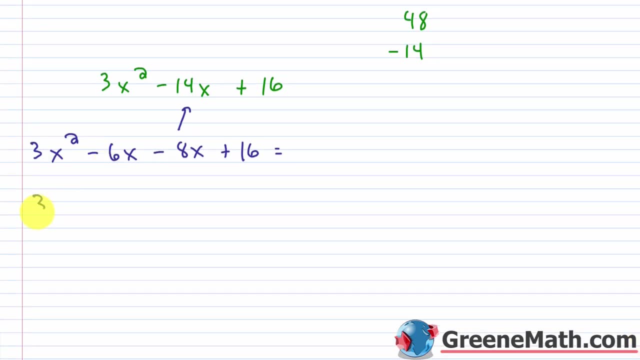 minus 8x plus 16.. We'll put this equals. Let me scroll down, get a little room going. From the first group: here I could pull out a 3x. I'm going to be left with x minus 2.. From the second group to match. 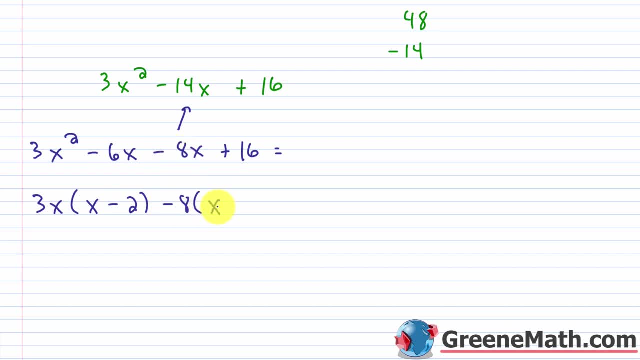 I'm going to pull out a negative 8. That would leave me with x minus 2. So I have that common binomial factor of x minus 2. And I want to bring that out. So if I factor that out, I have x minus. 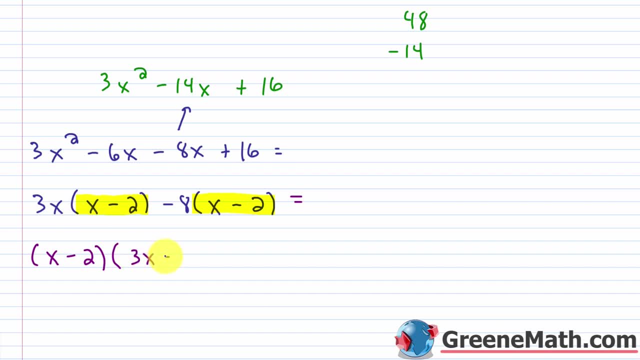 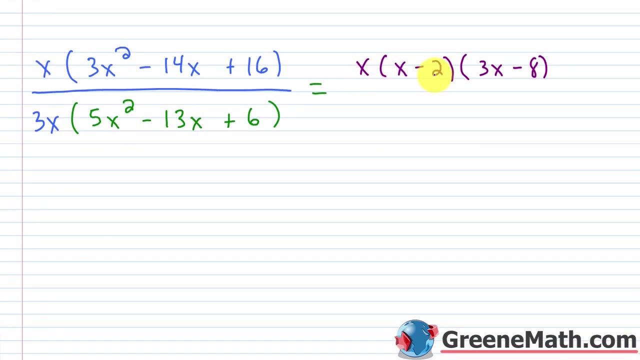 2, that quantity times a quantity 3x minus 8.. And so this is the factorization. So let me just copy this. So let's drag that up there. We have this x, that's outside. So we have x times the quantity x minus 2 times the quantity 3x minus 8.. That's your numerator. 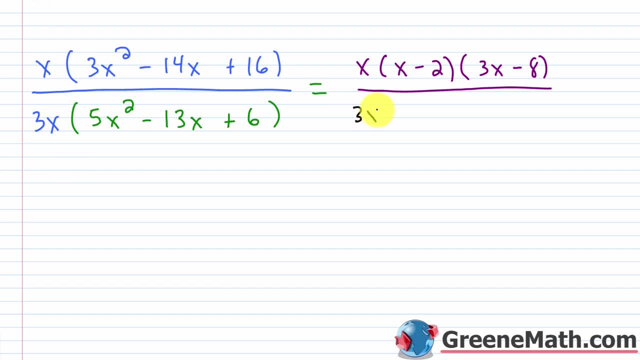 Now let's work on the denominator. So I have my 3x and then 5x squared minus 13x plus 6.. Let's factor that, So I want two integers whose product is 5 times 6 or 30 and whose sum is negative 13.. 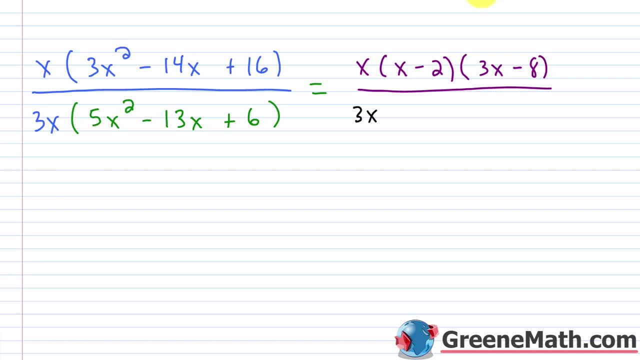 That one's really easy. You do negative 10 and negative 3. So you would have 5x squared minus 10x, minus 3x plus 6.. Again, I just use these two integers to rewrite that middle term. So then I'm going to factor by grouping, So from the first group I could pull out 5x. 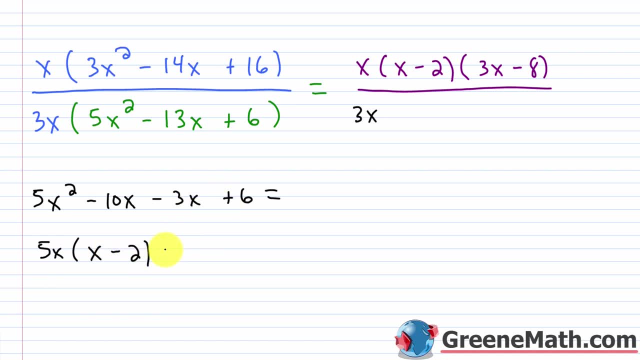 I'd be left with x minus 2.. From the second group I could pull out a negative 3 and I'd be left with x minus 2.. So I have that common binomial factor of x minus 2.. And so what that's going to give me is the quantity x minus 2 times the quantity 5x. 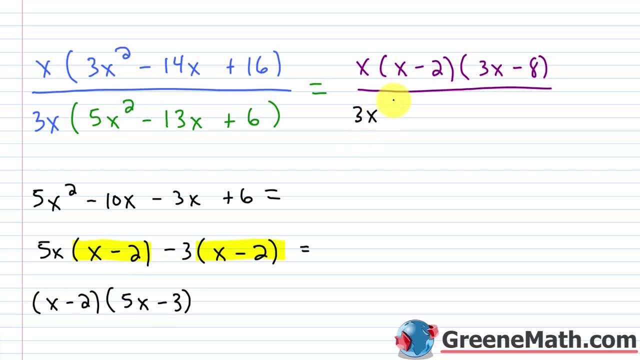 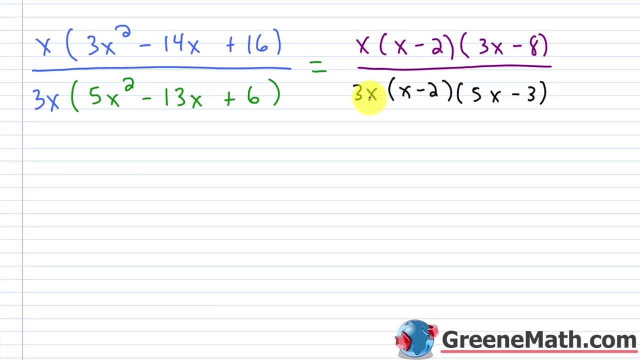 minus 3.. So I'd have 3x times the quantity x minus 2 times the quantity 5x minus 3.. All right, so let's erase all this. If I wanted to know the restricted values before I cancel anything, I would set this: 3x times the quantity x minus 2. 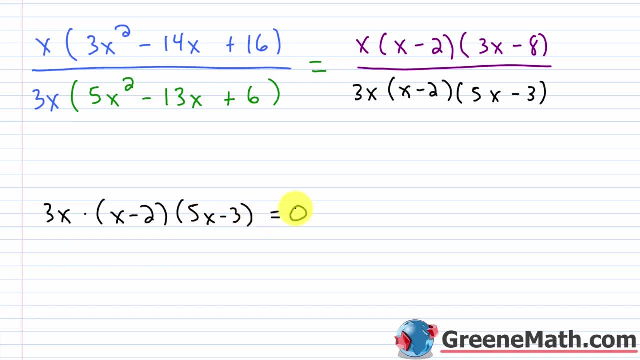 times the quantity 5x minus 3, equal to 0. And I'd use my zero product property to get a solution. Now you can do that if you want. You'd find your restricted values, Because once we start canceling things, you're going to lose information. 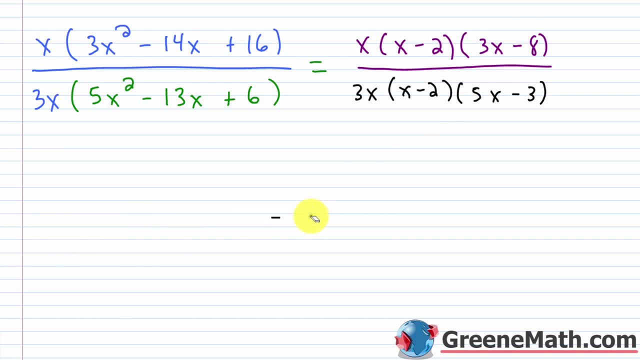 You're going to lose information. So if you're asked to do a simplification and also to find the restricted values, here's where you would do that. You would find the restricted values and then you would cancel afterwards. So, between the numerator and denominator. 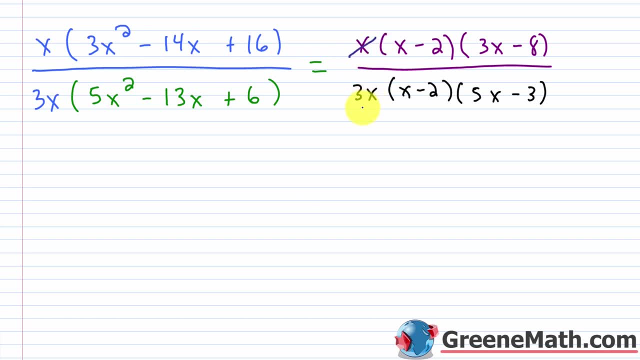 what are the common factors? We see that we have an x here that we can cancel with an x here. Then we have the quantity x minus 2. That cancels with the quantity x minus 2.. So what I'm left with this is gone. I have 3x minus 8.. 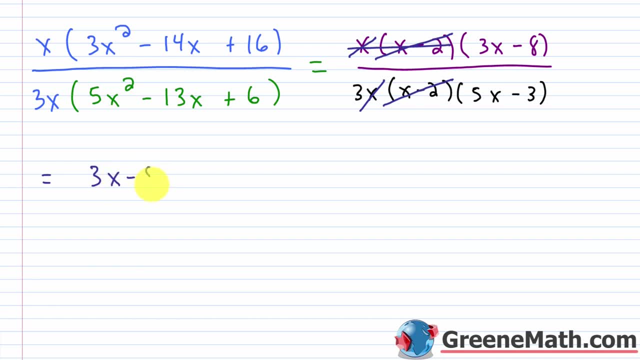 So no need to keep it inside of parentheses: 3x minus 8.. Then over Now we have 3 times, 3 times the quantity 5x minus 3.. And we keep this one inside of parentheses because this is multiplication. here And again, don't make the mistake of going and saying: well, I can cancel. 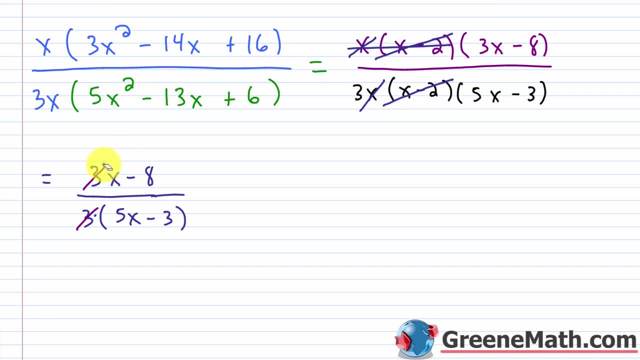 this 3 with this 3.. I'm going to cancel this 3 with this 3.. I'm going to cancel this 3 with this 3.. You can't do that, OK, It doesn't work that way. This is multiplication here, So these two are: 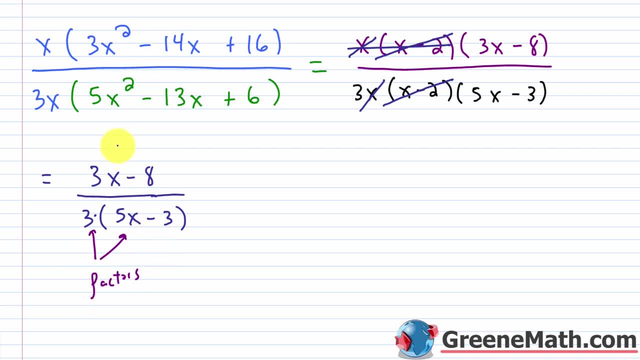 factors. But up here this 3x and this negative 8, those are not factors, That's a subtraction problem. So if I had 3x minus 8 multiplied by 3 like that, well then I can cancel this 3 with. 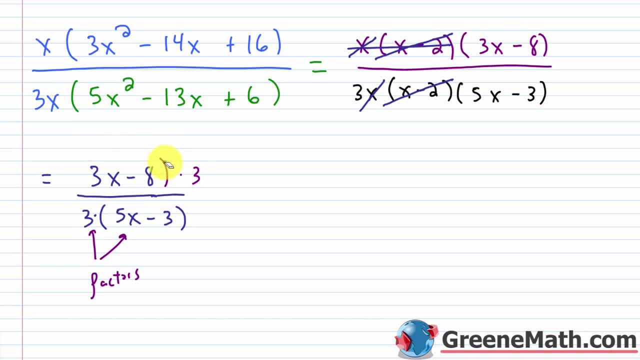 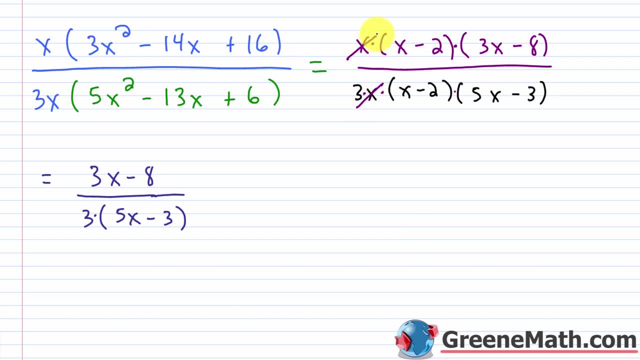 This is multiplication, So this cancels with this. Those are common factors And this cancels with this. Again, those are common factors. So in the numerator I'm just left with this, which is what I got: 3x minus 8.. In the denominator I'm still left with a 3 multiplied by the quantity. 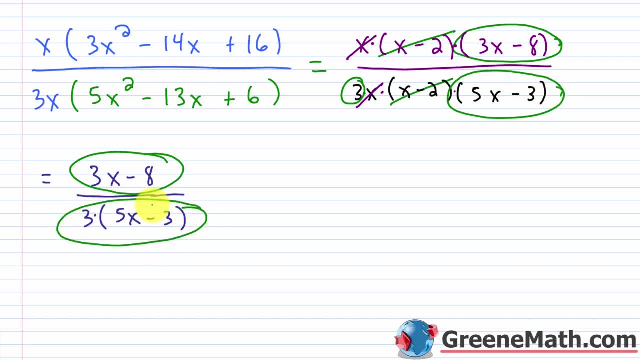 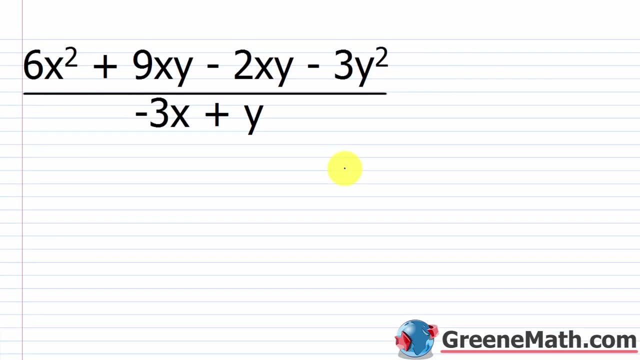 5x minus 3, which is what you have down here. So you end up with 3x minus 8, over 3 times the quantity 5x minus 3.. All right, let's take a look at one more problem. So we have 6x squared plus. 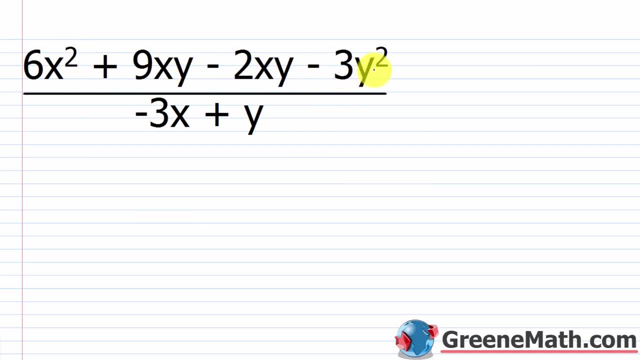 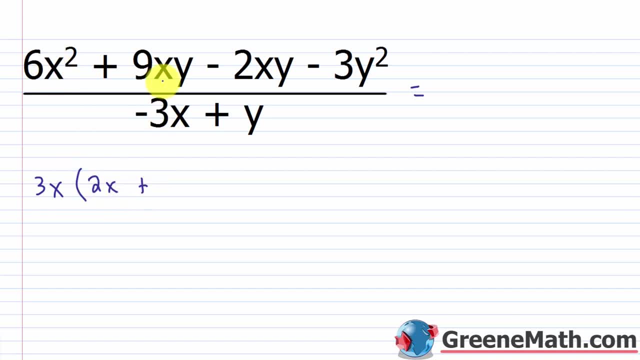 What I'd have left is a 2x plus a 3y. In the second group I could pull out a negative and then y, So what I'd have left is a positive 2x and then a positive 3y, so plus 3y. 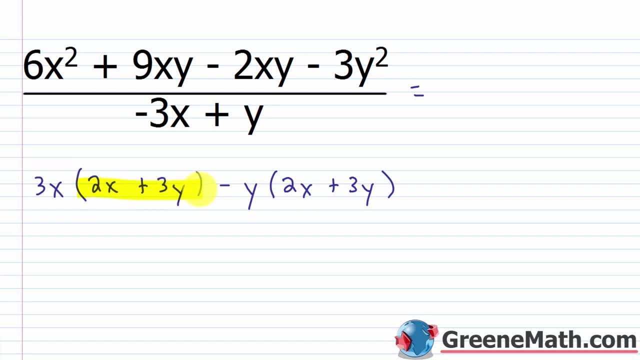 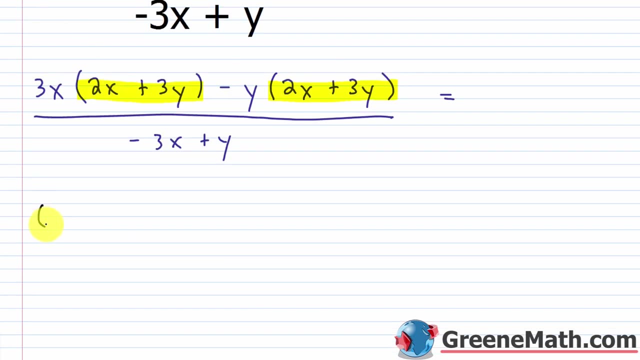 So you can see that you have a common binomial factor of 2x plus 3y. So let's put this equals in the denominator. I still have negative 3x plus y and so let's go ahead and factor this so I pull out that common binomial factor in the numerator. I'll have the quantity 2x. 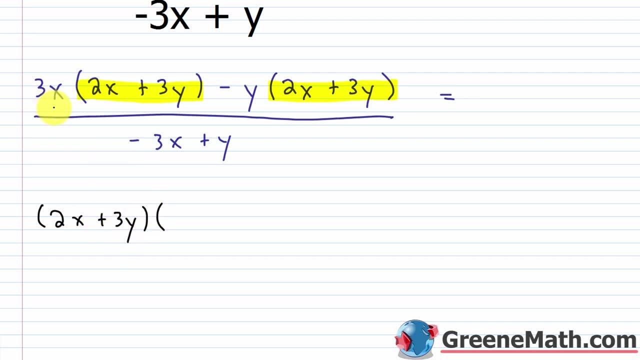 plus 3y, then times the quantity, you'll have 3x minus y and this is over. you have a negative 3x plus y. this 3x minus y looks similar to negative 3x plus y. the signs are just different. when the signs are different, but you have the same terms, they end up canceling and becoming. 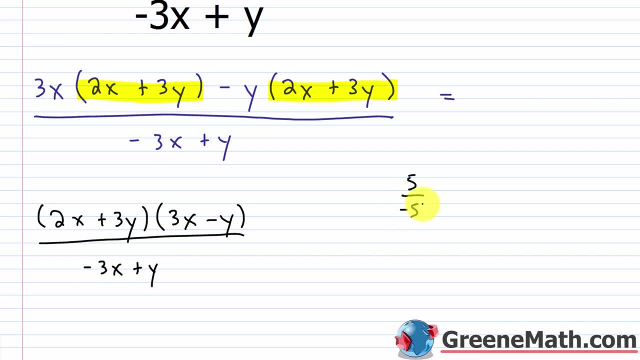 negative 1. it's kind of like having 5 over negative 5. it's the same thing, they're just opposites, so these would cancel, become negative 1. so it's the same concept here. and to prove that to you, what I'm going to do is I'm going to enclose this inside some parentheses. 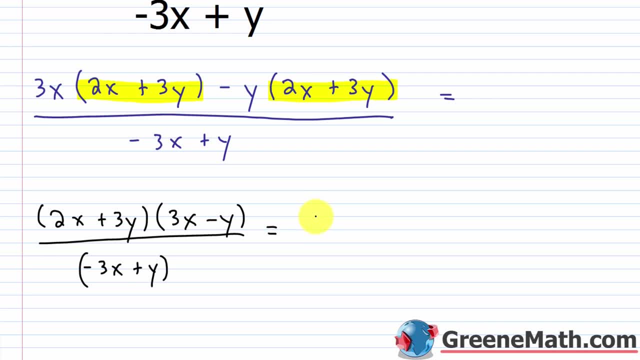 and I'm going to factor out a negative one. So keep the numerator the same. You have the quantity 2x plus 3y times. this is multiplication, the quantity 3x minus y. So each one is a factor. So this is a factor and this is a factor Now in the denominator, if I pull out a negative one. 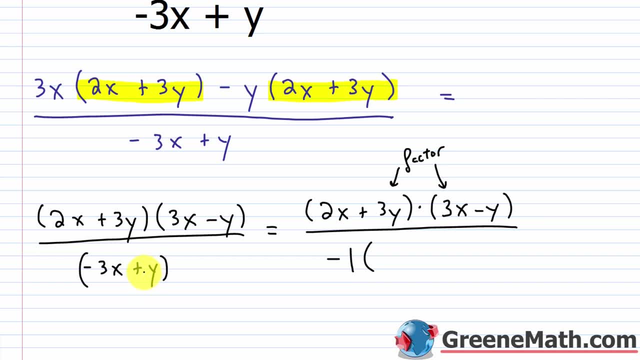 so I put a negative one out in front of parentheses. the signs would just change. So this would be 3x and then this would be minus y. So from negative 3x it becomes 3x, from positive y it becomes negative y. Now this is multiplication, So negative one is a factor. 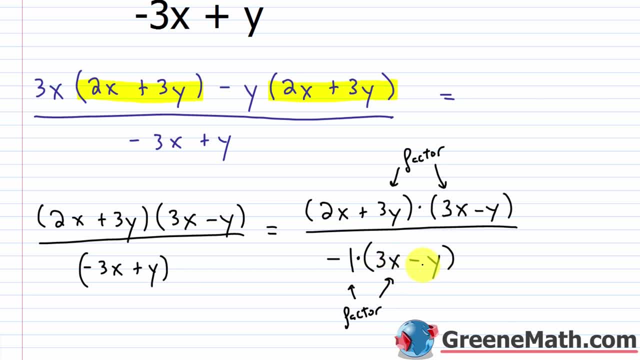 and so is the quantity 3x minus y. Inside of parentheses it's being multiplied. Now it is completely obvious, when I cancel this with this, that I'm left with this and I'm left with that negative one. So if you need to do that a few times for it to make sense, 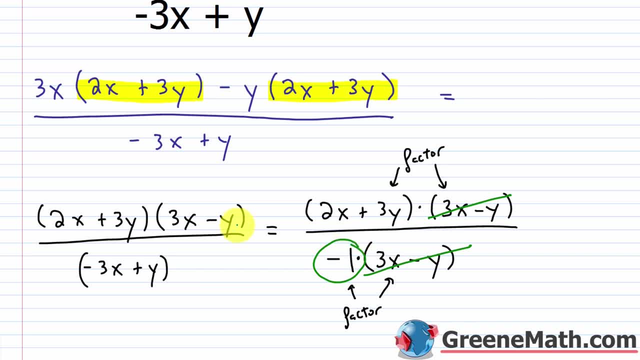 for you. go ahead and do it. But the quicker thing to do is to realize that if I have this and I have this, if I cancel them, I'm going to get negative one. You have 3x and negative 3x. 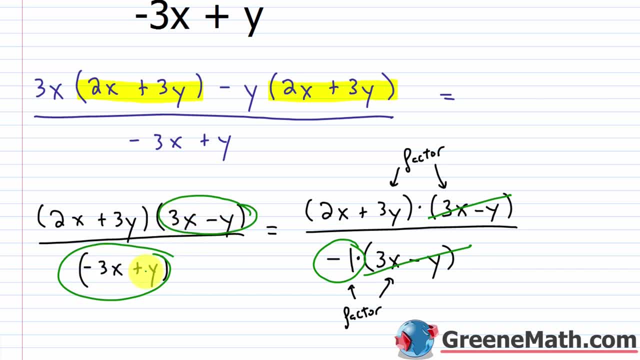 So basically, the same thing with the sign is different. You have negative y and positive y. same thing with the signs are different. So if you cancel that, you're going to end up with negative one. So my results here, my results here in the numerator: I'm just going to have that 2x. 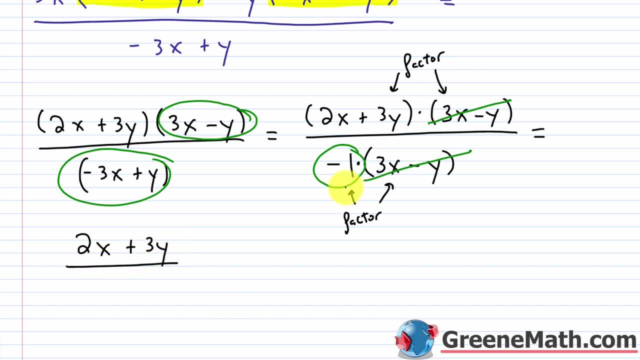 plus 3y In the denominator I have a negative one, So I can put over negative one. But if we divide by negative one, really I don't need the fraction bar anymore and get rid of that. I can put a negative one out in front like this, or I can just use the distributive property and say I have 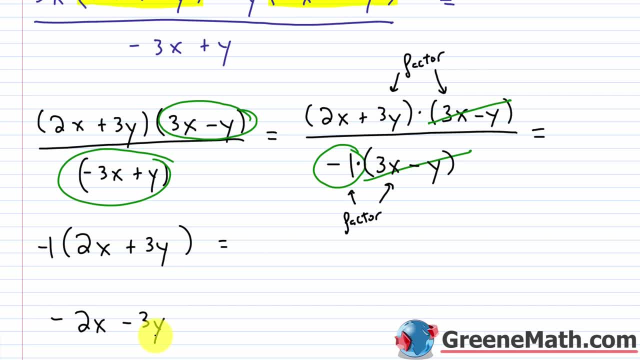 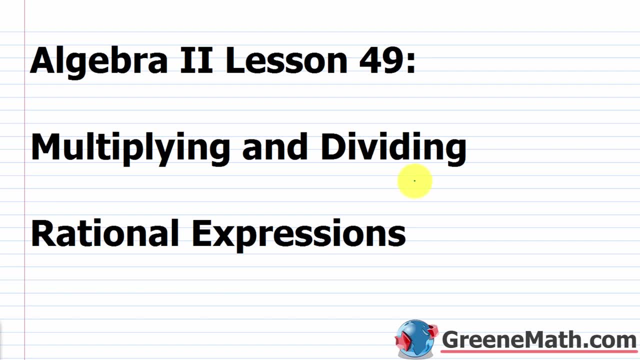 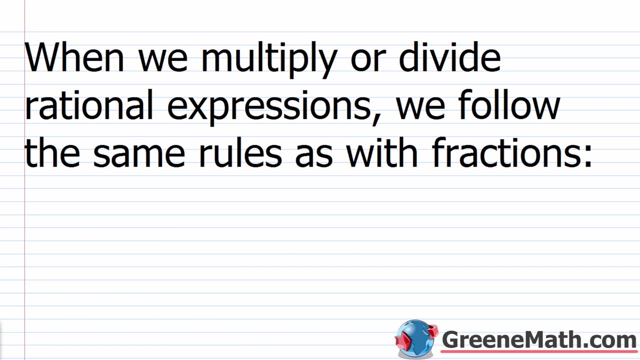 negative 2x minus 3y as my answer. Hello and welcome to Algebra 2, Lesson 49.. In this video we're going to learn about multiplying and dividing rational expressions. So again we've come across a topic that we learned back in Algebra 1, but we want to review. 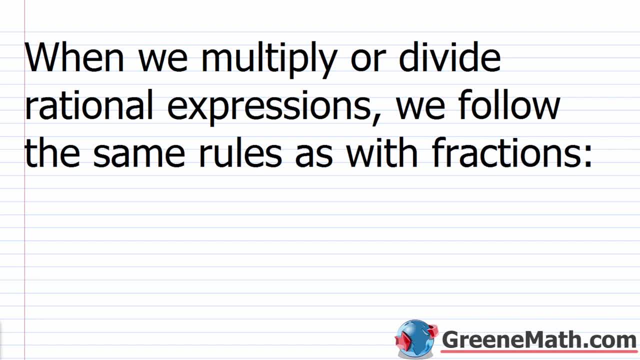 this for the purposes of Algebra 2.. Before we get into anything more complicated, we've got to make sure that we understand these topics that we learned in Algebra 1.. So I want to start by saying that when we multiply or divide rational expressions, we follow the same rules as with 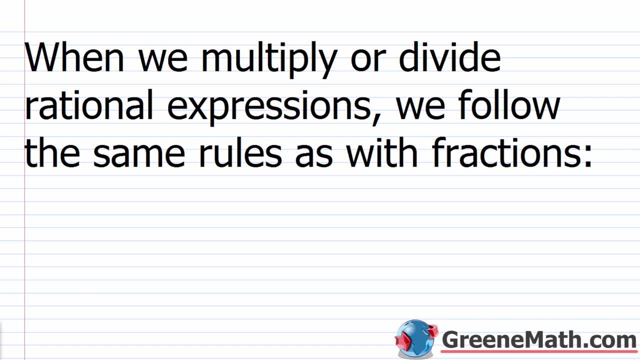 fractions. So if I was to multiply two fractions together- let's say it was something like one fourth times, Or let's say four sevenths- Well, we would check between the fractions to make sure that they were simplified first, And if they are, then I would check to see if I could cross cancel. I can cancel. 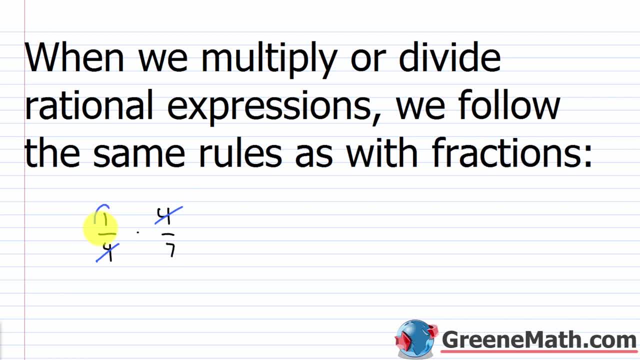 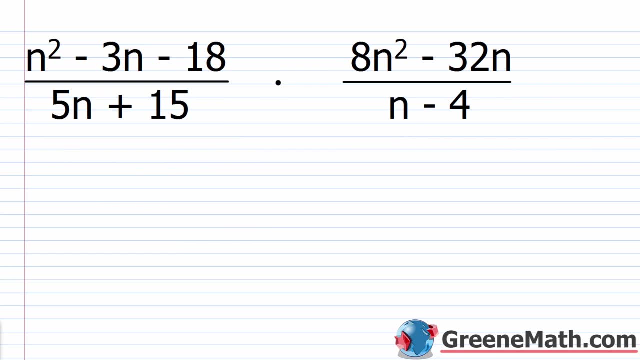 this four with this four. So that leaves me with just a one and a seven. So I'd have one over seven or one seventh as my answer. It's essentially the same process we're going to follow when we start multiplying and dividing rational expressions. So, as an example, let's say I had 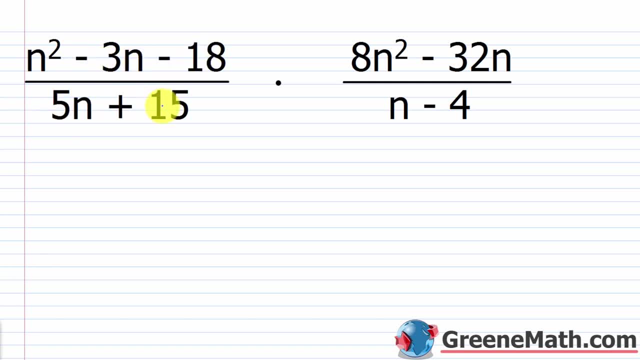 n squared minus 3n minus 18, over 5n plus 15.. And we multiply this by 8n squared minus 32n over n minus 4.. So the first thing I want to do is I want to factor everything completely. And when I factor, 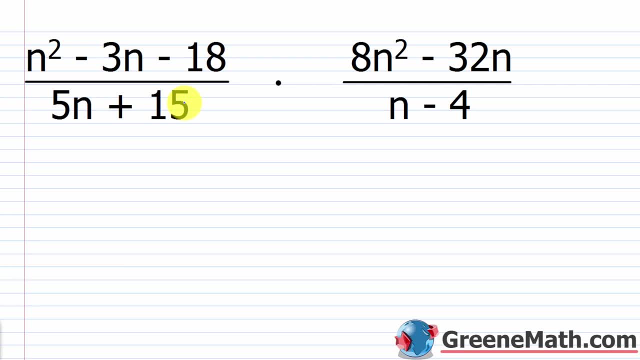 with these rational expressions. in a lot of cases it's going to work out to where you can cancel between numerator and denominator, and then I can also cross cancel as well. So let's just start out by factoring everything. So I'm going to put my equal sign. It's a factor n squared minus. 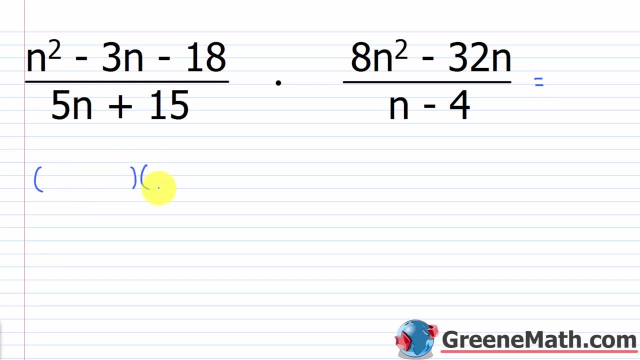 3n minus 18.. I can factor that into the product of two binomials. I know this would be n and this would be n, And then I need two integers whose sum is negative three and whose product is negative 18.. So we think about that. you'd come across negative six and positive three. Negative six. 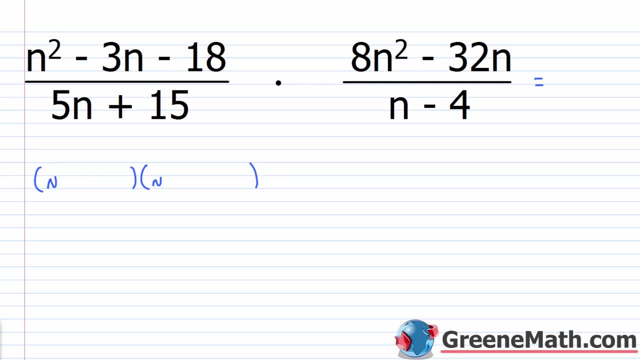 plus three would be negative three, And then negative six times three would be negative 18.. So we put negative six and positive three, And then negative six times three. would be negative six and positive three. All right, then we want to factor this guy right here. I would just look. 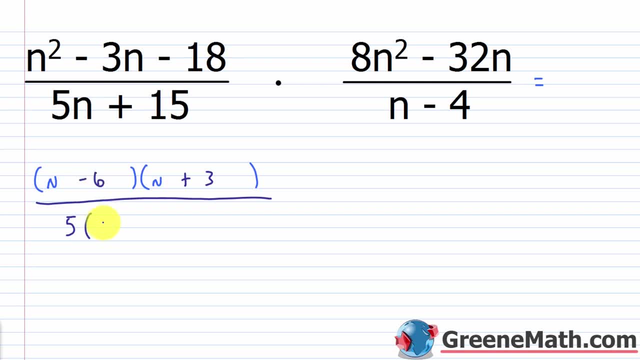 to pull out a five And that would leave me with what? An n plus three. So you can already see, before you go any further, that I can cancel this factor of n plus three with this factor of n plus three. Remember, this is multiplication, So these are factors, And these are factors, And we cancel. 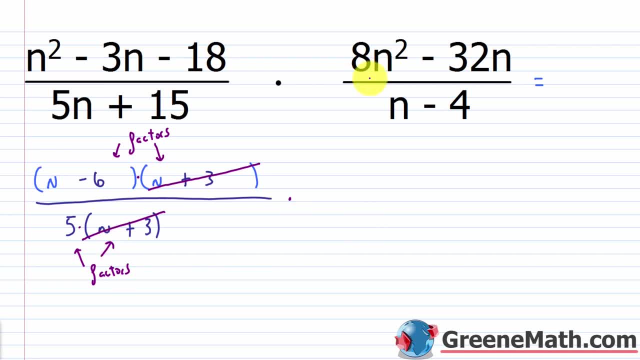 common factors. All right, then times Over here in the numerator I can start by pulling out an 8n, So I'd be left with n minus four, And then in the denominator I have n minus four, So you'll. 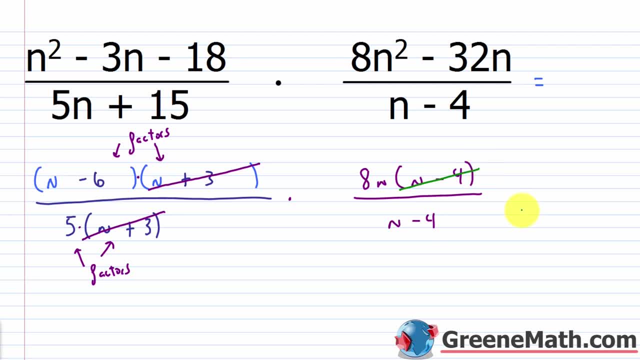 notice. you can cancel a common factor here of n minus four And to make that obvious, put this in parentheses and put times one, And then you'll realize: this is a factor And so is this. Or you can say: these are both factors, These are factors as well. 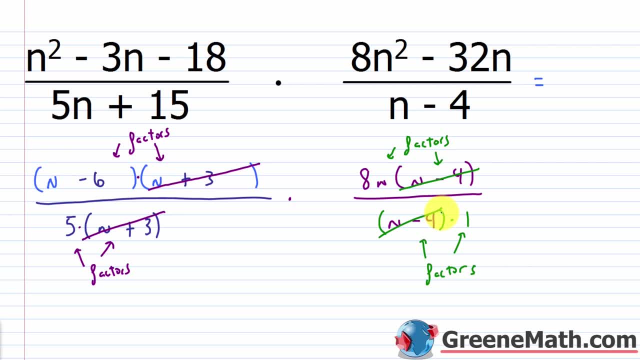 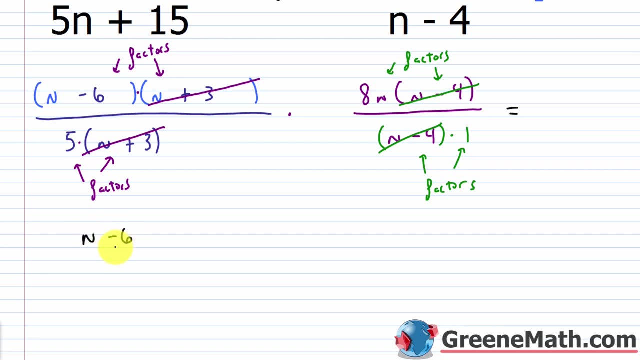 So you cancel those common factors, All right. so now that I have done that- I've canceled between numerator and denominator of each- I'm going to look to see can I cross cancel anything before I multiply. So let me just rewrite what's left. I'd have n minus six over five multiplied by 8n. 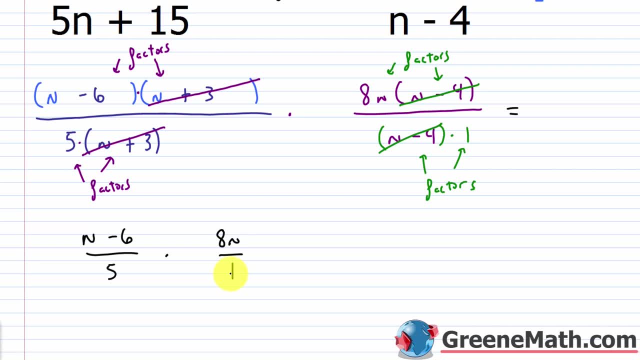 You could put over one if you want. So can I cancel anything between five and 8n? No, I cannot. Can I cancel anything between n minus six and one? No, I cannot. So I can leave this in factored form and say: this is 8n times the quantity n minus. 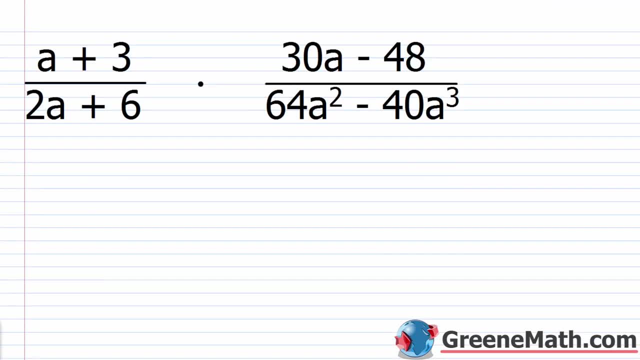 six over five. All right, let's go ahead and take a look at the next example. So we have a plus three over 2a plus six. This is multiplied by 30a minus 48 over 64a squared minus 40a cubed. So again, 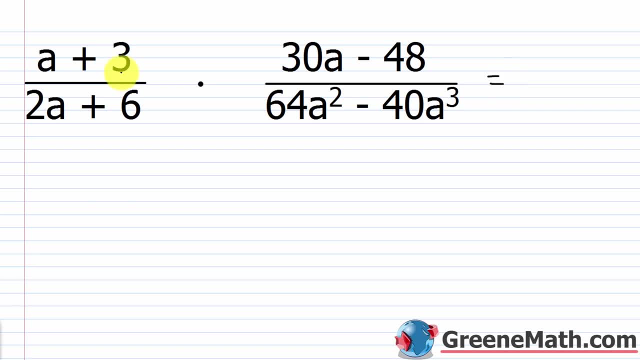 I just want to factor everything With a plus three. I cannot factor that, So I'm just going to leave it as a plus three. With this one, 2a plus six. you know you could pull a two out, So you'd have two times the. 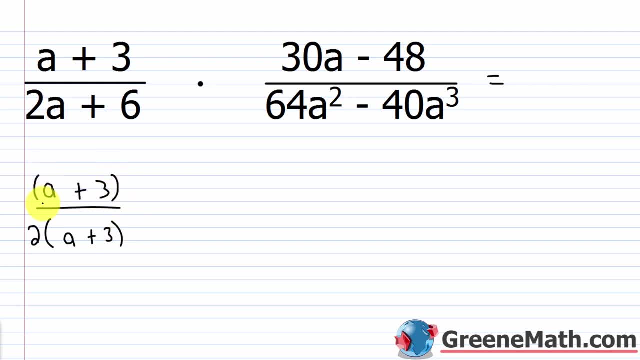 quantity a plus three. And obviously you can now cancel between the numerator and denominator this factor of a plus three. I'm going to put times one here, just to make that obvious for you that these are factors. Then times over here I have 30a minus 48.. So 30 and 48 share a common. 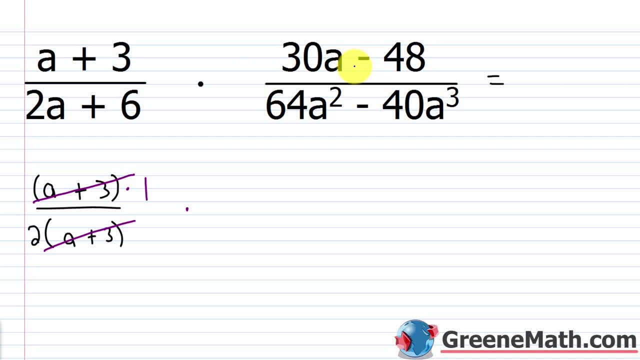 factor of two and also three. So that means that each share a common factor of six. So let's pull six out. That would leave me with 5a minus eight inside, And then the denominator: I have a 64 and I have a 40. So those are each divisible by four. They're also each divisible by eight. It's about: 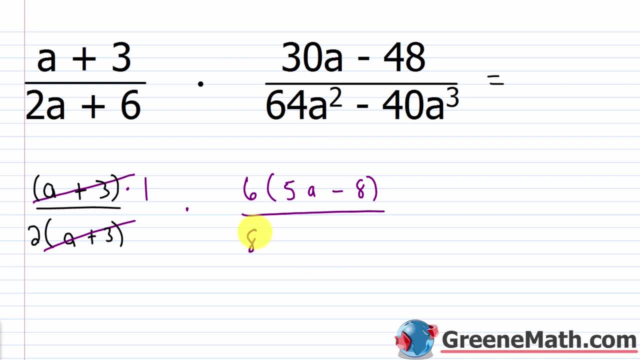 as best we can do. So let's pull out an eight, And then we have a squared and a cubed. So 8a squared is what we can pull out. So I'd be left with eight. Then you'd have your minus 5a Now. 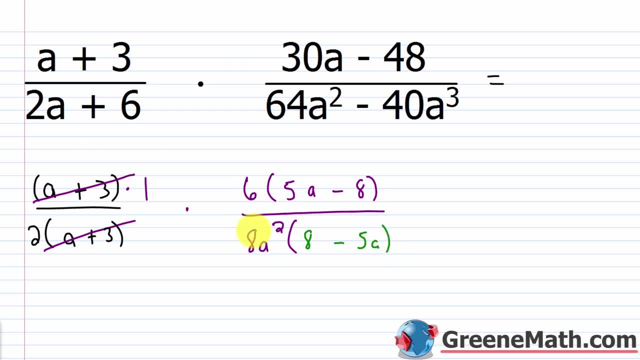 we know we can do some canceling between here and here, but let's hold off on that for a second. I have 5a minus 8.. I have 8 minus 5a. Those are opposites, If you'll notice. I have 5a. 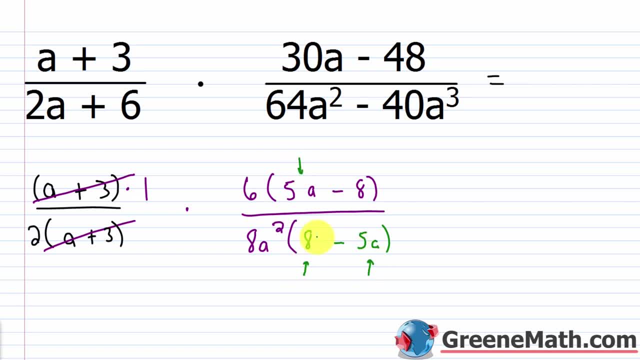 and I have 5a. Forget about the sign for a second. I have 8 and I have 8.. Each one has an opposite sign. Here 8 is negative. Here 8 is positive. Here we have negative 5a. Here we have positive. 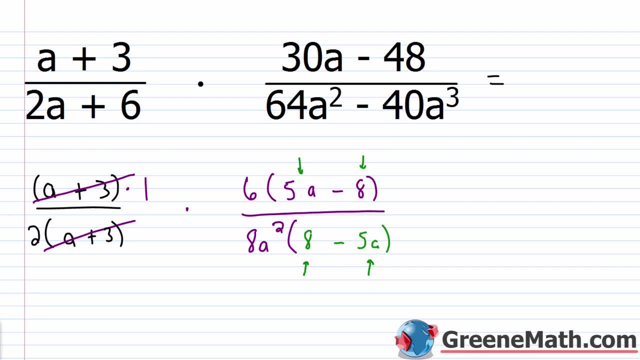 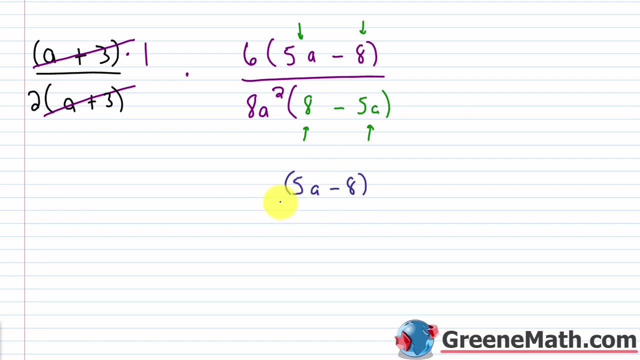 5a. So if you have opposites like that, essentially you can just cancel them and say the sign is negative 1. If I was to do a little side note here and just show you this, I could take this right here. Let me just start with 5a minus 8 and put it in parentheses. I'll just put times. 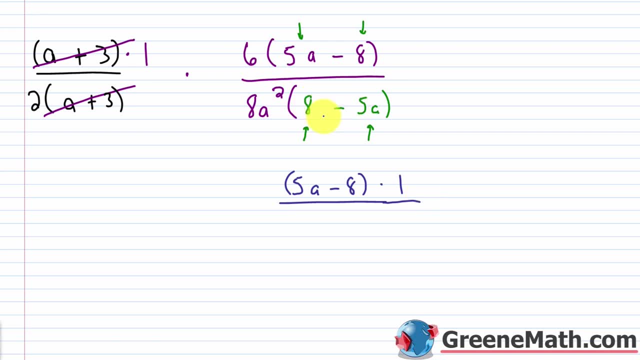 1 and make it completely crystal clear what's going on For this one, let's just rearrange the order. Let's say this is negative 5a plus 8, like this: Now let's say I factored out a negative 1. 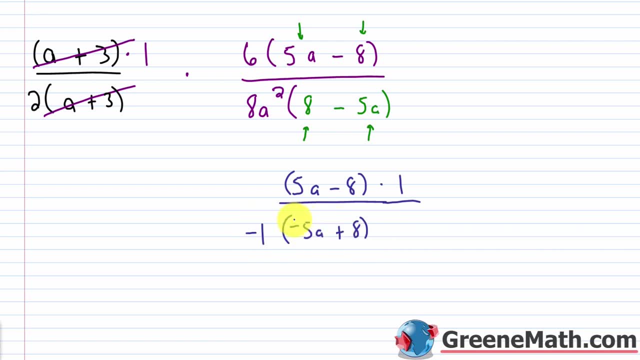 from here. So if I pulled out a negative 1, what would happen? This would turn positive And this would turn negative. So now we have 5a minus 8 and 5a minus 8.. This would cancel with this and leave me with this. I now have 1 over negative 1, which is just negative 1.. So again, 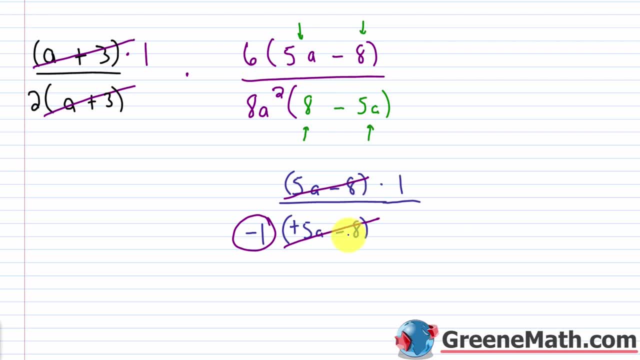 if you see that situation, you don't need to go through this long, lengthy process. I've got the same terms but with different signs. I know those are opposites, So I can cancel this with this and say it's a negative 1. Now I can do some more canceling if I want. 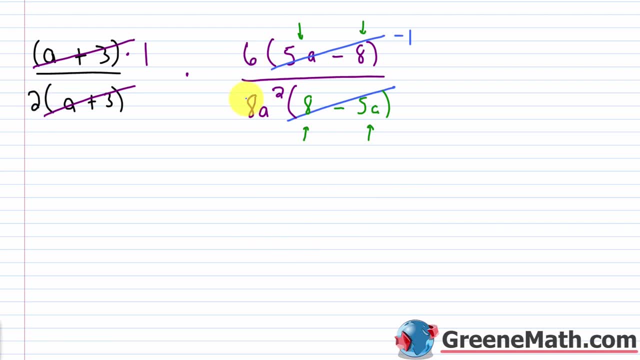 6 and 2 have a common factor of 2.. And I know 6 and 8 have a common factor of 2.. So whatever you want to cancel that with, it's up to you. It's going to be the same in the end. I'll just cancel. 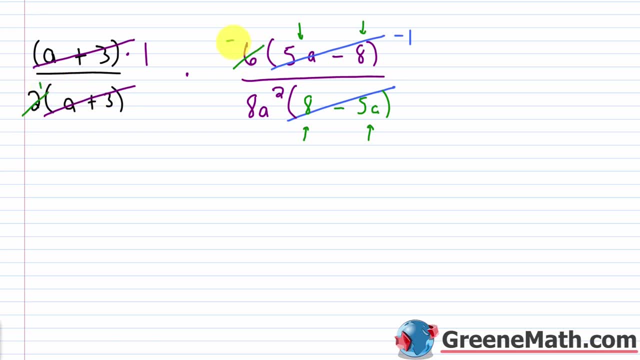 this 6 with this 2.. I'll say this is a 1 and now this is a 3.. So this right here is completely canceled. This is a 1. So I don't even need to worry about it. 1 times anything is itself. 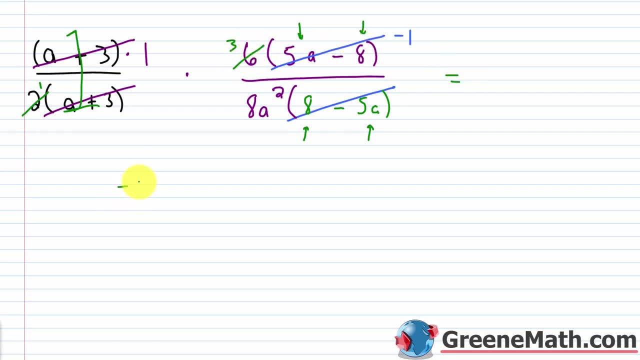 In the numerator here I have 3 times negative 1, which is negative 3.. In the denominator I just have 8a squared. So my answer here is negative 3 over 8a squared. Let's take a look at one more of these And then. 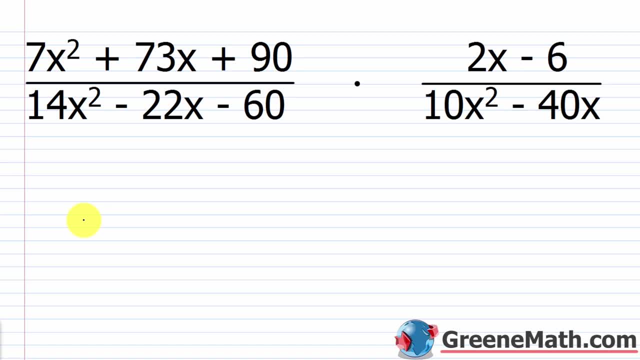 we're going to jump in and look at some division. I think you can see that it's pretty easy to do. It's just a lot of canceling, a lot of trying to get things simplified. All right, So we have 7x. 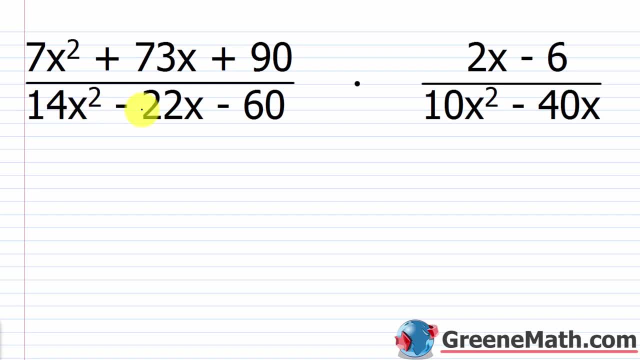 squared plus 73x plus 90 over 14x. squared minus 22x minus 60.. And this is multiplied by 2x minus 6 over 10x squared minus 40x. So the first thing I want to do is try to factor out the 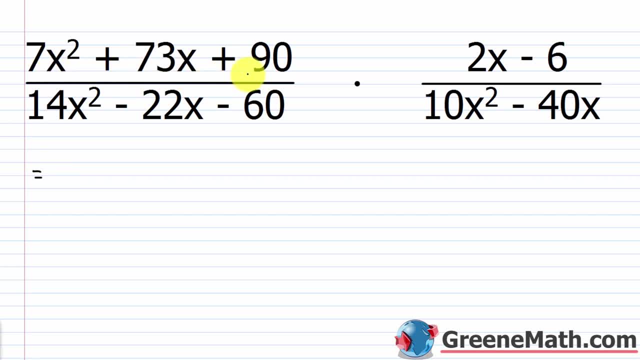 everything And for 7x squared plus 73x plus 90,, we can think about two integers whose product would be 7 times 90,, which is 630, and whose sum is 73. I know that two such integers would be. 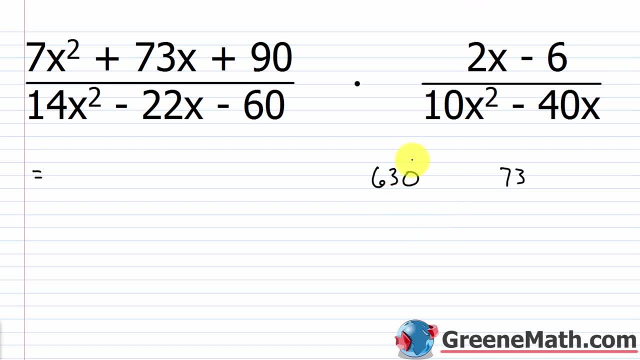 positive. Let's think about 630 for a second. It ends in a 0. So I know it would be 63 times 10.. Now 63 and 10 add to be 73. So I've found my two integers pretty easily. 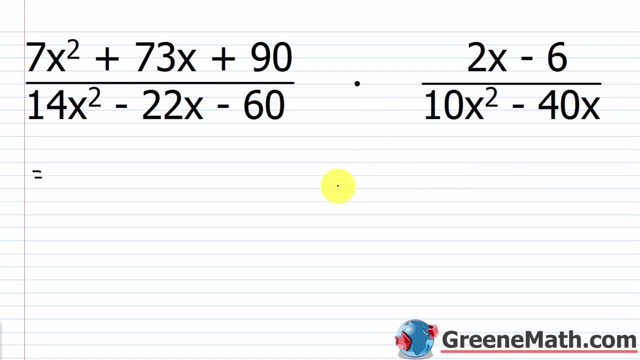 Let's erase this. I'm going to use those two integers to rewrite this middle term here. So I'm going to say that we have 7x squared plus. I'm going to say we have 63x plus 10x plus 90.. 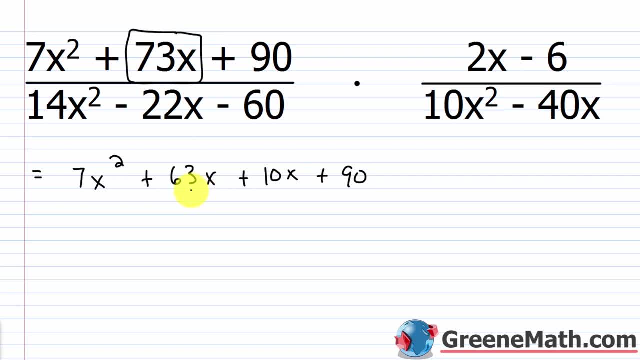 Again, I took this middle term 73x and I wrote it as 63x plus 10x. Didn't do anything illegal. Now I'm going to factor by grouping. So from the first group I could pull out a 7x. 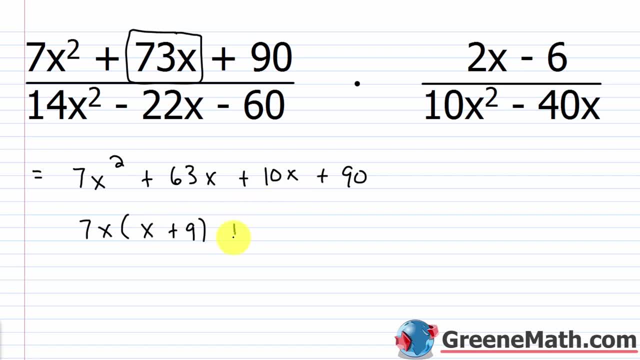 and I'd be left with x plus 9.. From the second group, I could pull out a 10, and I'd be left with x plus 9.. So I could factor out this common binomial factor of x plus 9.. 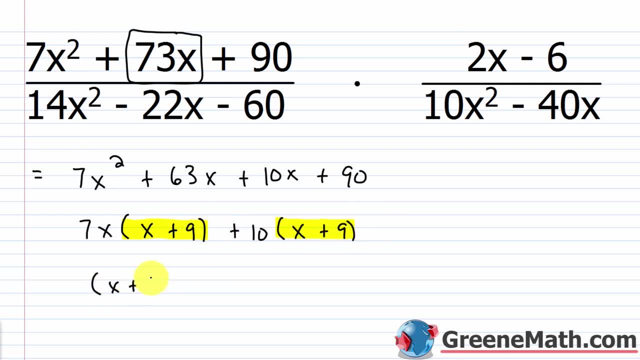 And what's that going to leave me with? I would have x plus 9, that quantity multiplied by the quantity 7x plus 10.. And so let me erase this and I'll write this in factored form: I've got x plus 9, that quantity multiplied by the quantity. 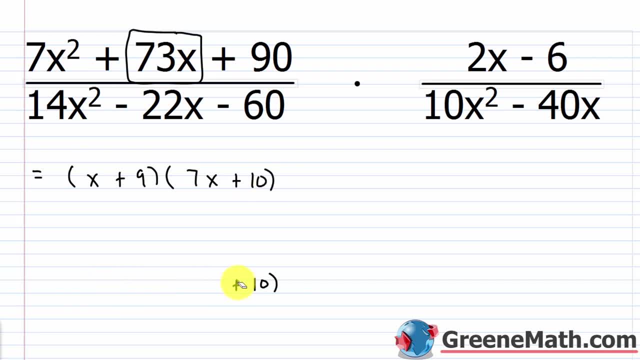 7x plus 10.. All right, so let's work on the denominator now. In the denominator, everything is even. so I could start by just pulling out a 2, and I'd be left with 7x squared minus 11x minus 30.. 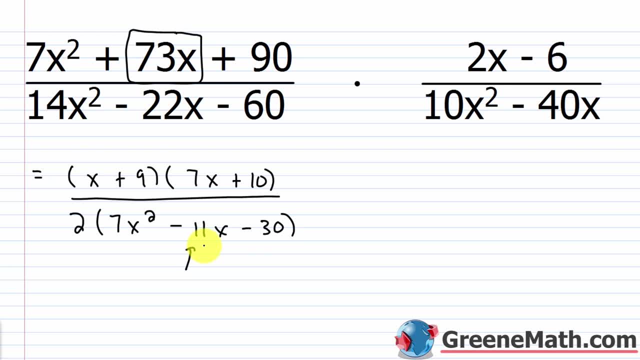 Now, how can we factor this? Well, give me two integers whose product is 7 times negative 30 or negative 210, and whose sum is negative 11.. Well, this is another one, If I just think about positive 210. for a second: 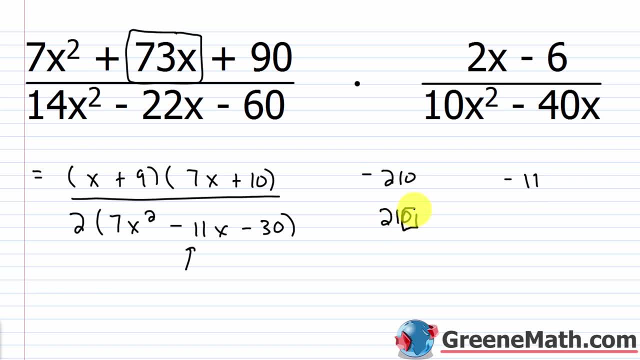 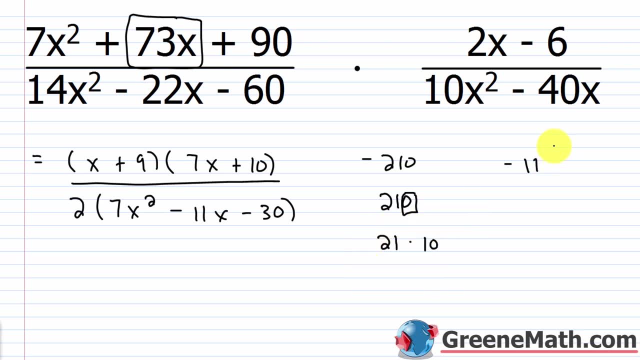 I just think about 210.. It ends in a zero, So I know it will be 21 times 10.. So I can play with the signs with 21 and 10, and get myself a sum of negative 11 and a product of negative 210. 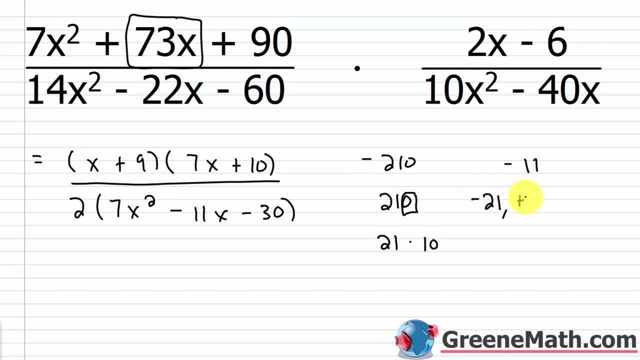 If I had negative 21 and positive 10, that would do it for me. Negative 21 times positive 10 is negative 210.. Negative 21 plus 10 is going to give me negative 11.. So let me go ahead and factor this. 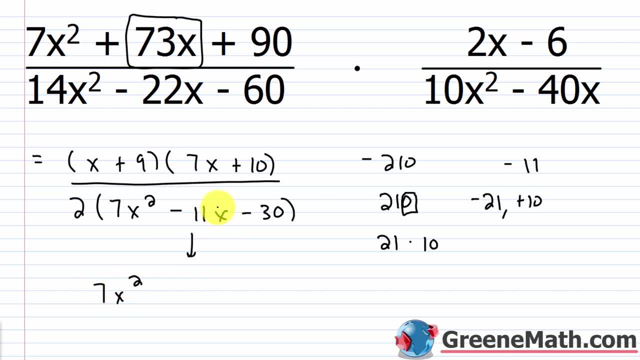 part down here. If I had 7x squared, I'm going to rewrite the middle term using these two, So minus 21x and then plus 10x and then minus 30. So let me scroll down for a minute. I'll come. 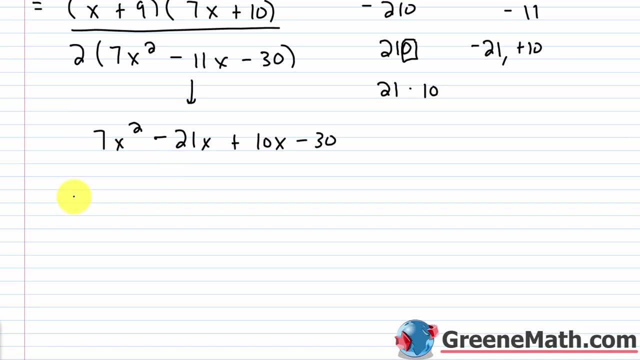 right back in a second. So from the first group I could pull out a 7x. I'd be left with x minus 3 inside. From the second group, I could pull out a 10 and I'd be left with x minus 3 inside. 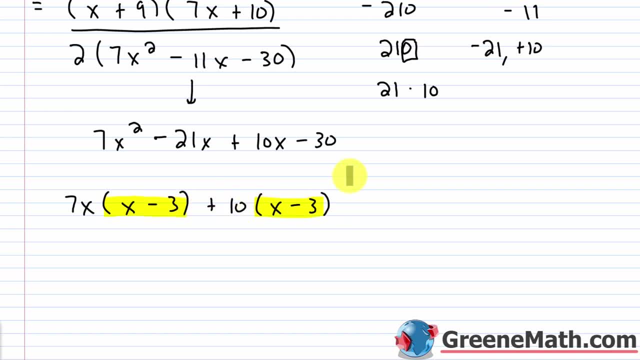 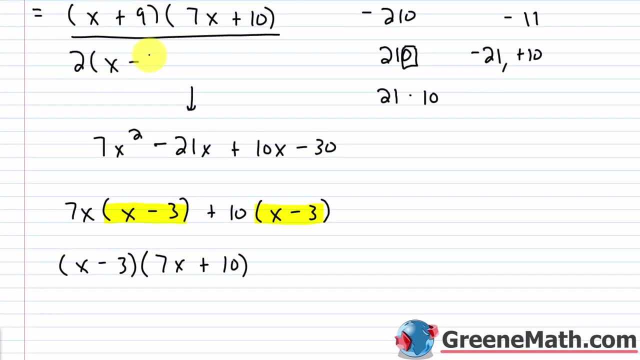 So I would factor out this common binomial factor of x minus 3, and that would give me the quantity x minus 3 multiplied by the quantity. You'd have 7x then plus 10.. All right, So let's erase this part. We'll have 2 times the quantity x minus 3. 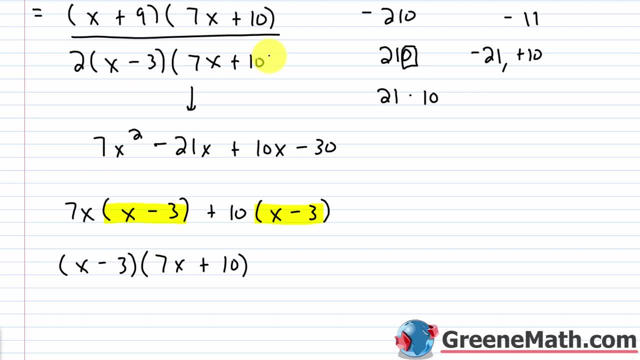 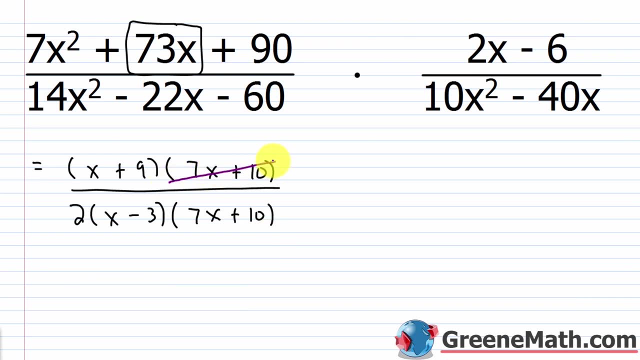 then times the quantity 7x plus 10.. All right, So let's erase all this And we can see that we can cancel a common factor of 7x plus 10.. That's canceled. Remember, this is multiplication. Those are all factors, So 2x plus 10.. 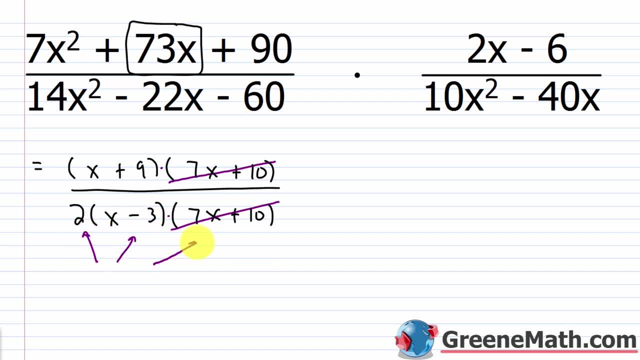 The quantity x minus 3 is a factor And the quantity 7x plus 10 is a factor. These are factors. And then the quantity x plus 9 is a factor, And then the quantity 7x plus 10 is a. 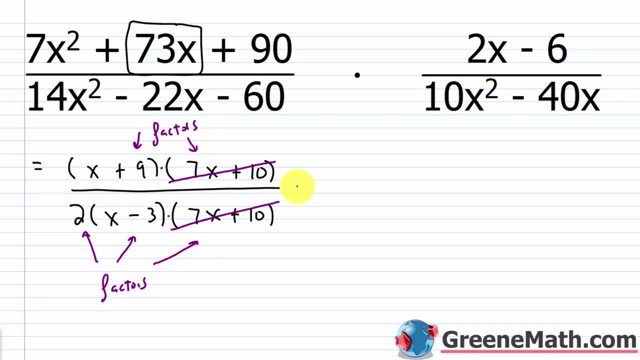 factor. So we canceled common factors Then times. For these guys it's going to be easier to factor: Pull out a 2 from the first one, So I'd have x minus 3 inside In the denominator. here I could pull out a 10x And I'd be left with 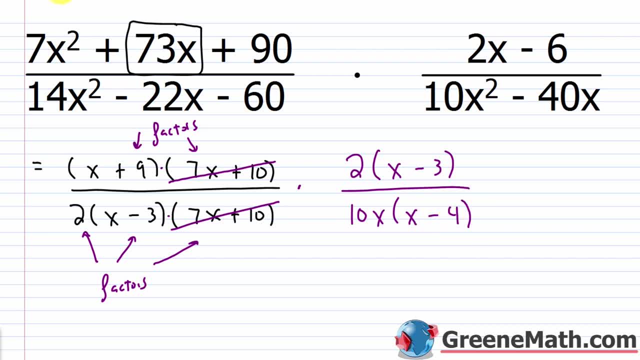 x minus 4 inside. So what can I cancel here? Well, I know, between 2 and 10, I can cancel a common factor of 2.. So this would be 5.. I can now cross cancel a factor of x minus 3 between here. 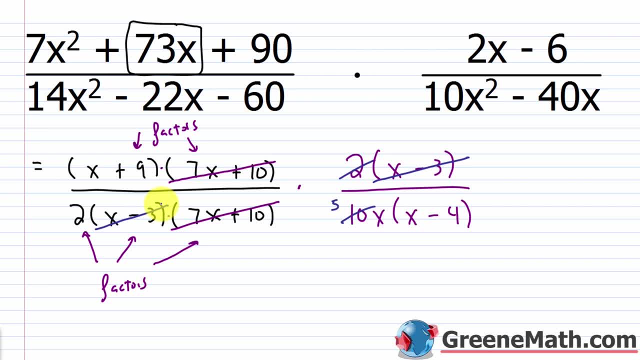 and here. So that's gone And nothing really else that I can do. I have x plus 9 here. Nothing to cancel with that in my denominator or the denominator over here. This is completely canceled, So really nothing else I can do. 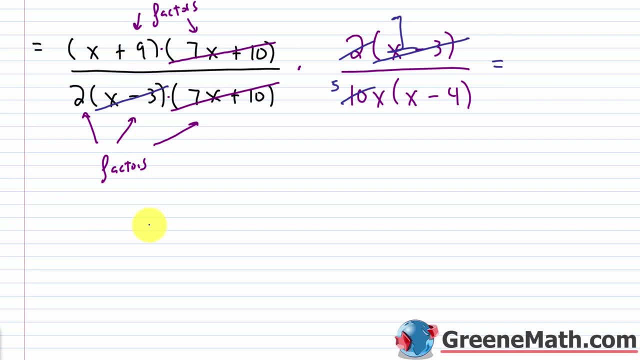 So let's just put equals. We have x plus 9 for our numerator, that quantity In the denominator, we have 2 times 5 times x, which is 10x times the quantity x minus 4.. And again, I'm just going to leave this in factored form because this is generally preferable. 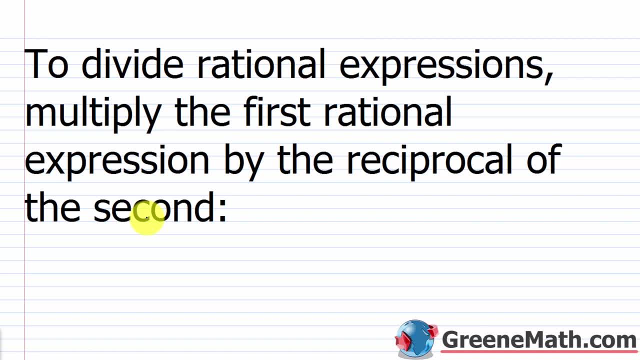 All right. So the next thing we want to talk about would be dividing rational expressions. So to divide rational expressions, multiply the first rational expression by the reciprocal and that means we flip it of the second. All right For the first problem. 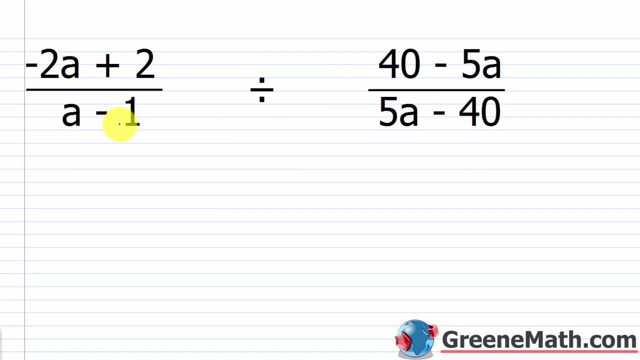 we're looking at negative: 2a plus 2 over a minus 1. And this is divided by: we have 40 minus 5a over 5a minus 40. So if I look over here, what can I factor? Well, I can factor out a negative. 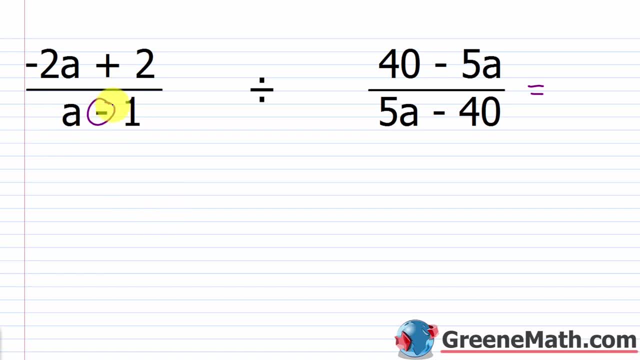 2 or a positive 2.. Because this sign here is negative, let's go ahead and factor out a negative 2.. That's going to leave me with a minus 1 inside Down. here I just have a minus 1.. If you want, you can enclose this inside of parentheses and put times 1 so that it's crystal. 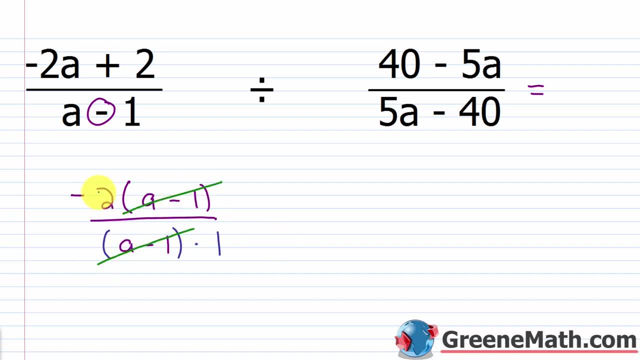 clear that you can cancel this with this. I'm left with negative 2 over 1 there. Then this is divided by. so that means I'm going to multiply by the reciprocal of this. So that means 5a minus 40 would come up to the numerator 5a minus 40, and 40 minus 5a would go into the denominator. 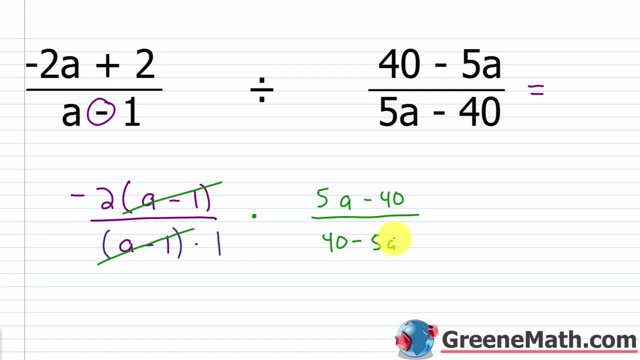 Now, before I go through and factor anything, what do you notice here? I have 5a and negative 5a. I have negative 40 and positive 40. These two are opposites. And again, if you want to switch, 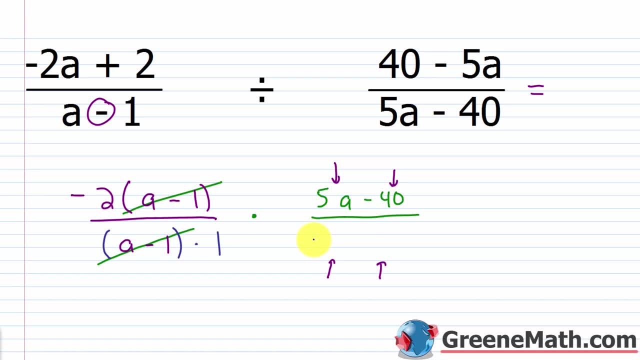 the order around and say this is negative, 5a plus 40, like that, and then factor out a negative 1 from one of them, it doesn't matter which one. If I factor out a negative 1, then I would erase. 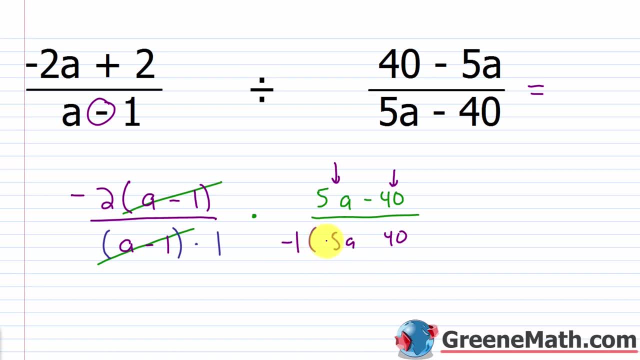 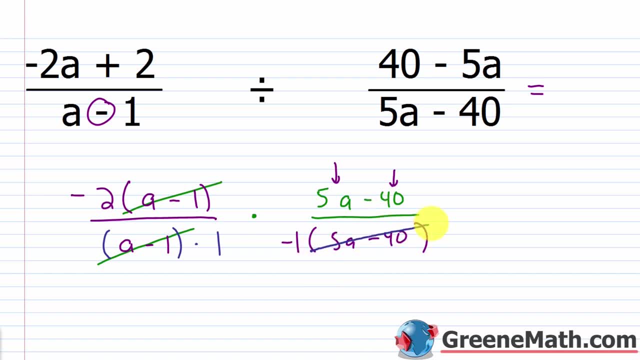 So that would get me back to what I had. So now, when you look at these two, it's obvious that this cancels with this. I can put it inside of parentheses and put times 1, if you want, And what I'm left with is 1 over negative 1, or just negative 1.. So what I get for my answer here. 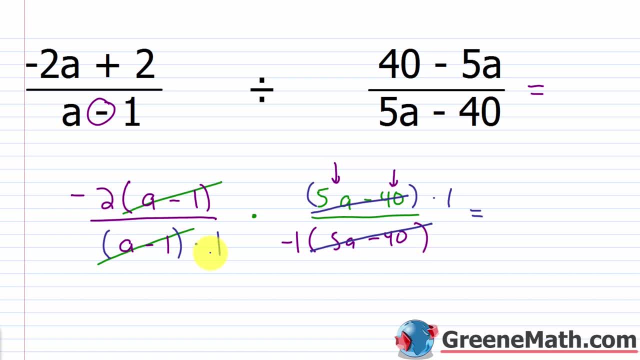 I have negative 2 over 1,, which is just negative 2, multiplied by 1 over negative 1.. I'm left with negative 2 over 1,, which is just negative 2, multiplied by 1 over negative 1,. 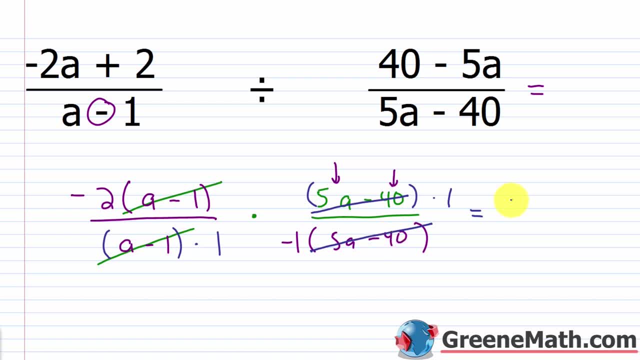 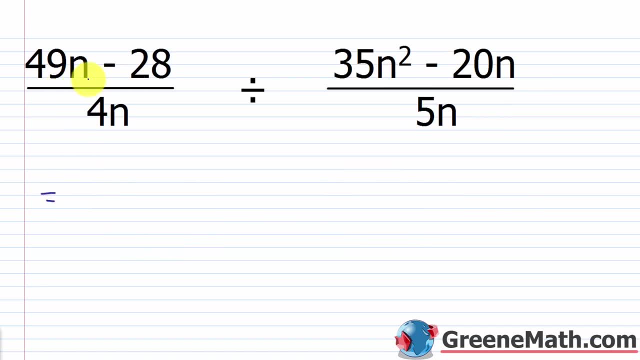 which is negative 1.. So negative 2 times negative 1 is simply 2, and that's my answer. All right, let's take a look at another one now. So what we're going to do here, I'm going to factor the numerator of this first guy and it looks like I could pull out a 7.. 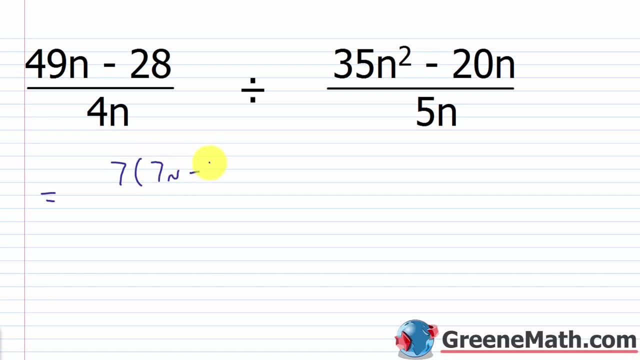 So if I pulled out a 7, I'd be left with 7n minus 4.. This is over 4n, And then I'm dividing by, so I want to multiply by the reciprocal. So bring 5n up here and this is over. 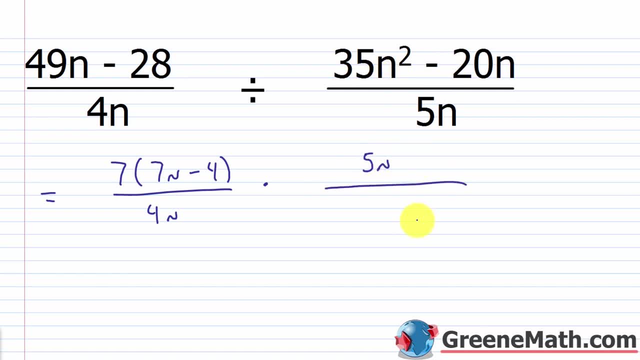 From this numerator. here it's going into the denominator, but I want to just go ahead and factor it. I can pull out a 5n, So I pull out a 5n and I'd be left with 7n minus 4.. 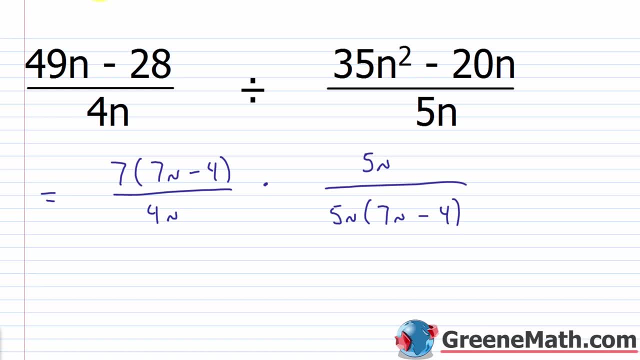 So now, what can I do? Well, it's obvious that I can cancel this 5n with this 5n, and I can cancel this quantity 7n minus 4 with this quantity 7n minus 4.. So this has canceled and become 1.. So all I'm really left with is 7 over 4n. 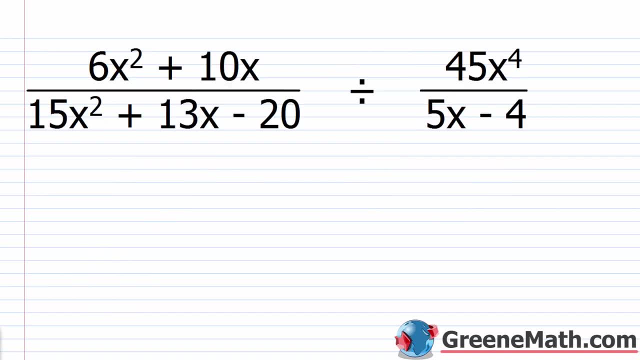 and so that's going to be my answer: 7 over 4n. Let's take a look at one more problem. So we have 6x squared plus 10x over 15x squared plus 13x minus 20.. 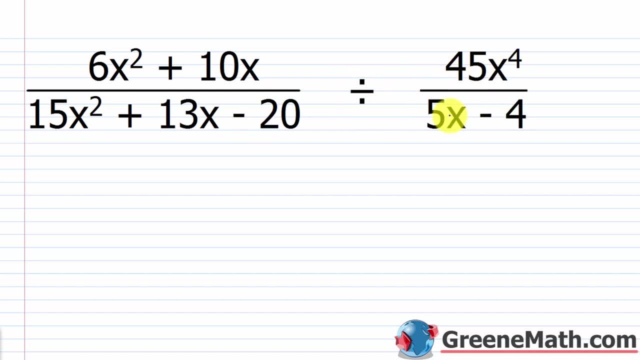 This is divided by 45x to the fourth, power over 5x minus 4.. All right, so from the numerator of the first fraction here I know I could pull out a 2x, So that would leave me with a 3x plus a 5.. 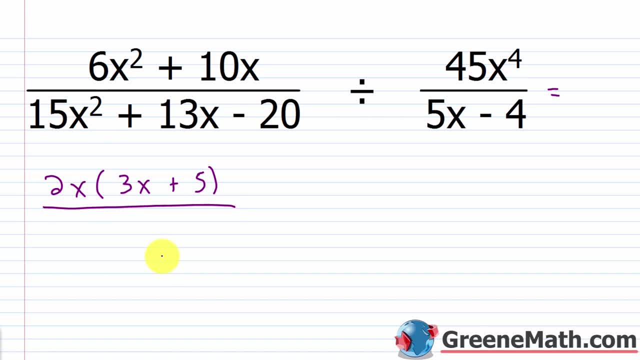 And the denominator of the first fraction here. I know I could pull out a 2x Down here. I can't start by factoring anything out. 13 is a prime number. Nothing's going to be common, So I'm going to try to factor this using grouping. So 15 times negative 20 is negative 300.. 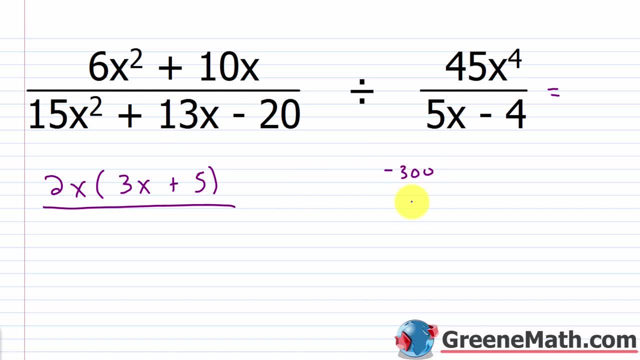 So I want a product of negative 300 and a sum of 13.. So a sum of 13.. All right, think about factors of 300. Let's just think about 300 for a second. I know they're going to have to be somewhat close together because it's going to be a sum of 13.. 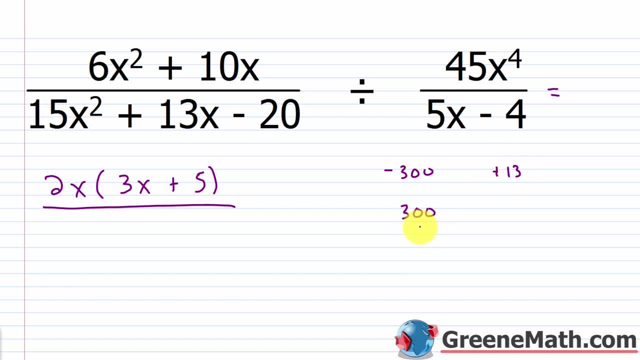 So I'm going to exclude things like 1 times 300 or 2 times 150.. I want to get kind of closer together. So if I just cut this off and say I know it's 30 times 10, I could work from there. Okay, now, 30 and 10 won't work, but I can decrease this one. 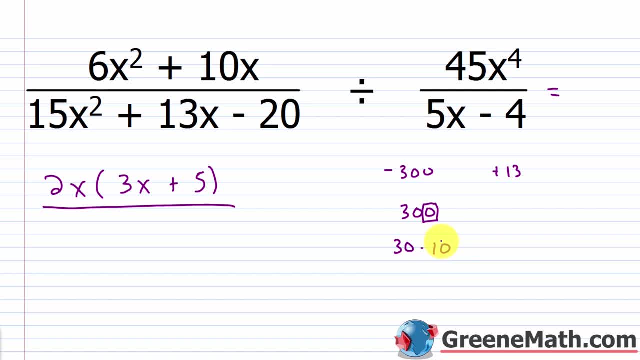 and increase this one. So the next two factors would be 25 times 12.. Now, 25 and 12, if I play with the signs- can produce a positive 13 as a sum and a negative 300 as a product. I would want positive 25 and negative 12.. So let's use that to rewrite that middle term. 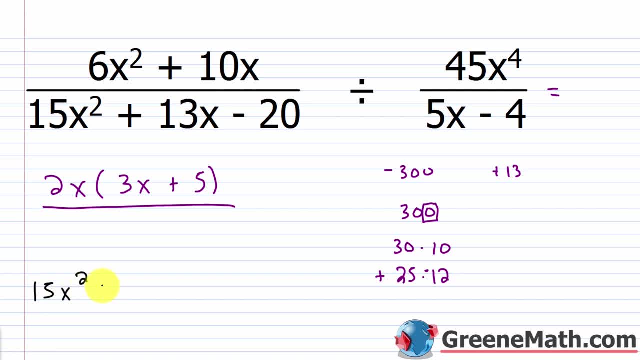 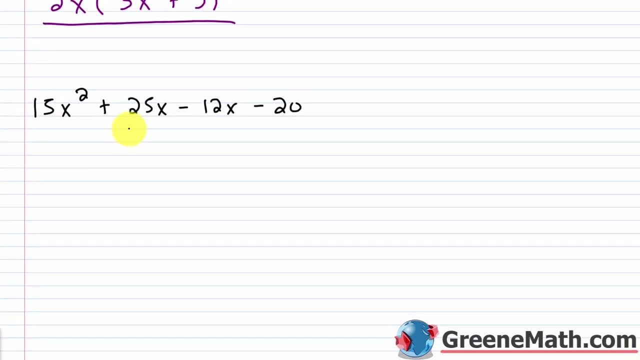 So we're going to say this is 15x squared plus 25x, minus 12x minus 20.. Let me erase this so we have a little bit of room to work And I'll scroll down a little bit. So from the first group here I could pull out a 5x. That would leave me with 3x plus 5.. 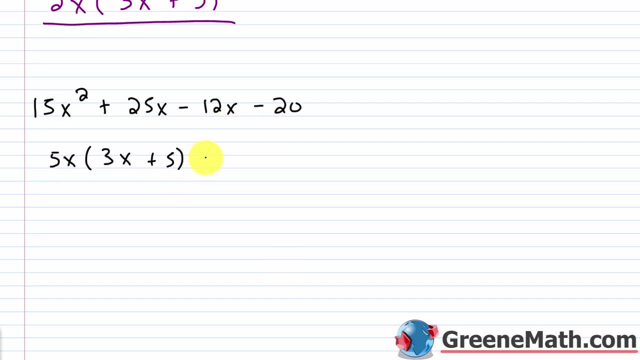 From the second group, I could pull out a negative 4.. Both signs here are negative. Both signs here are positive. So that's why I'm pulling out a negative along with that 4.. So that would leave me with 3x plus 5 inside, And so I have a common binomial factor of 3x plus 5.. 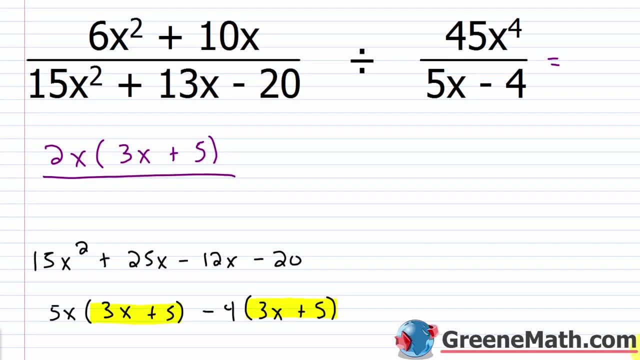 So let's go ahead and factor this out. So I have a common binomial factor of 3x plus 5.. So let's go ahead and factor that out And we'll just write our answer above. So we'll have 3x plus 5, that quantity Multiplied by the quantity we have, 5x and then minus 4.. 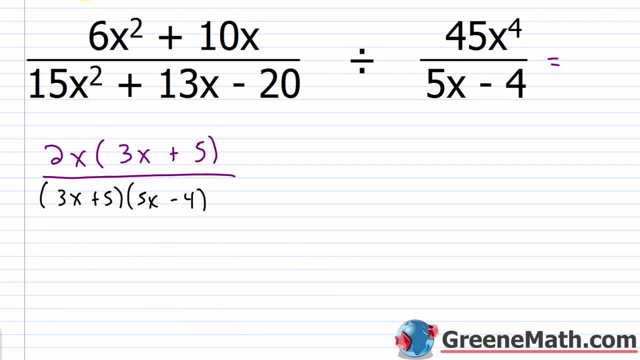 So let's erase all this, And we can already see that we could cancel this factor of 3x plus 5 with this factor of 3x plus 5.. Nothing else to cancel between numerator and denominator here. Then we're going to multiply by the reciprocal of this, So 45x to the fourth power would go. 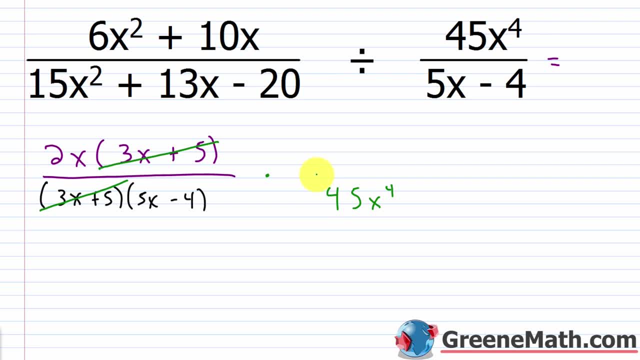 into the denominator. So we're going to multiply by the reciprocal of this. So 45x to the fourth power would go into the denominator. Nothing I can really do with that. In the numerator I just have 5x minus 4.. Nothing I can really do with that Now. what I can do is I can cancel this with this. 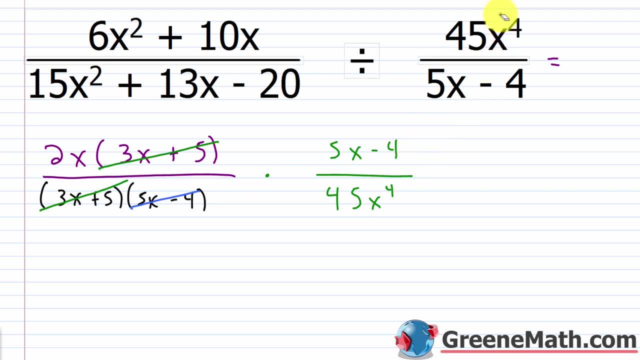 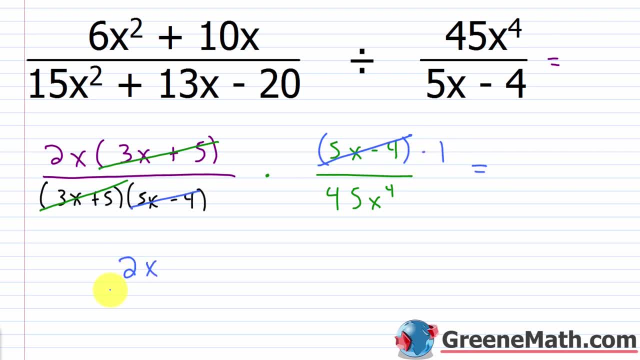 times 1, or just 2x over 45x to the fourth power. Now can I simplify this any further? Yeah, I can cancel one of these x's. This would be x to the third now, with this x here Between 2. 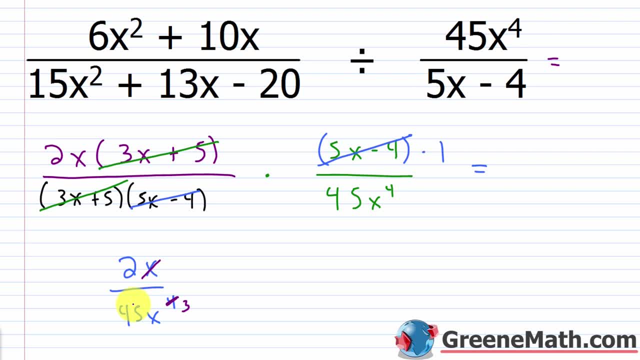 and 45, there are no common factors other than 1.. So I really can't do anything with that, So we'll end up writing this as 2 over 45x cubed. Hello and welcome to Algebra. 2.. I'm your host. 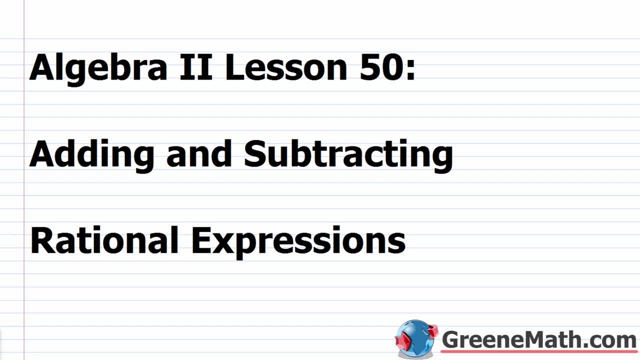 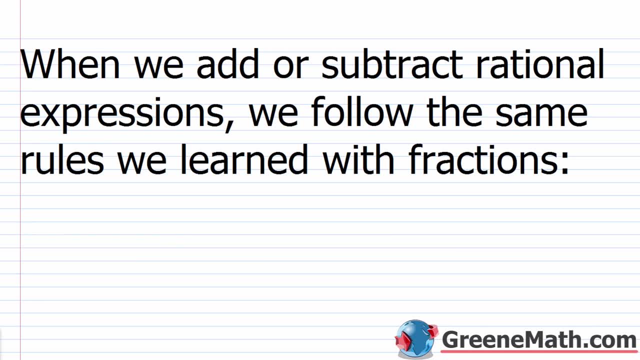 Lesson 50. In this video we're going to learn about adding and subtracting rational expressions. So again we've come across another lesson that we talked about back in Algebra 1.. So we should at this point have a fair understanding of how to add and subtract rational expressions. If you 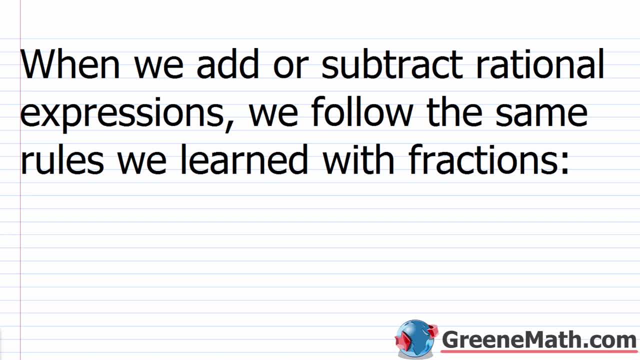 don't. you can pick it up from this lesson. We're just going to go a little bit quicker. In Algebra 1, we had two separate lessons. We first talked about how to find the LCD for a group of rational expressions, And then we moved into a lesson where we talked about how to add and subtract. 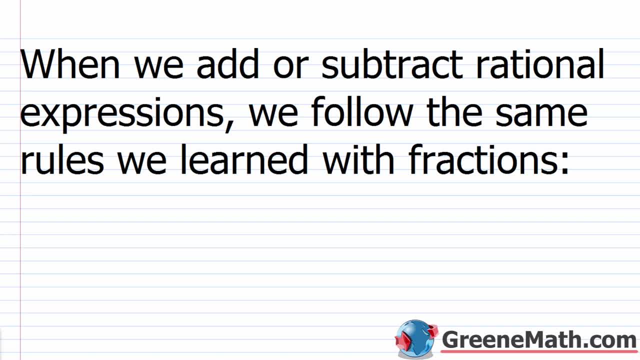 rational expressions. Here we feel like you have enough understanding of this. It's just a review, So we're going to compact it into one lesson. So I have here: when we add or subtract rational expressions, we follow the same rules we learned with fractions. So essentially, when the 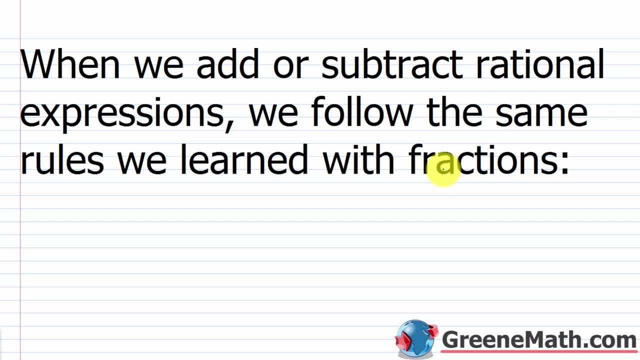 denominators are the same. you just add the numerators and place the result over the common denominator. So we're going to add or subtract rational expressions And then we're going to add 1 plus 3.. So if I had something like one fourth plus, let's say, three-fourths, I have a common 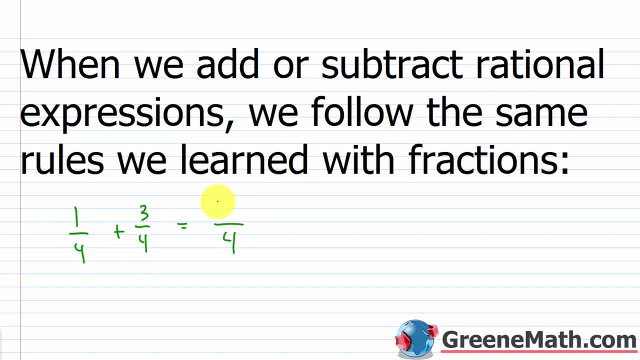 denominator 4, so that stays the same, And I add one plus 3,, which is 4.. And then the thing you want to, whatever you're done, is simplify. We know 4 over 4 is 1, so we would simplify that Now. 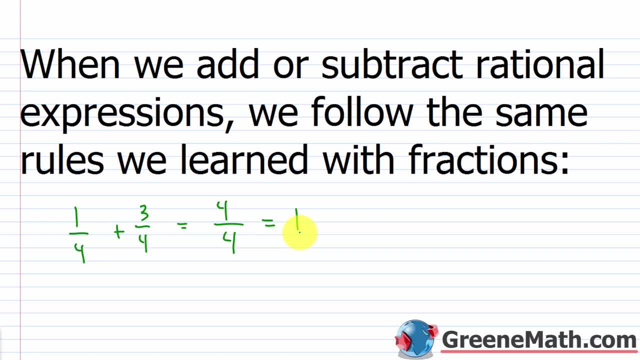 the other scenario, the more difficult or challenged scenario, is when the denominators are different. So the first thing is you have to find the LCD And then you get to the denominator of the tree, So longer then the core of a tree. you need to subtract and subtract while they are in Dortmund. 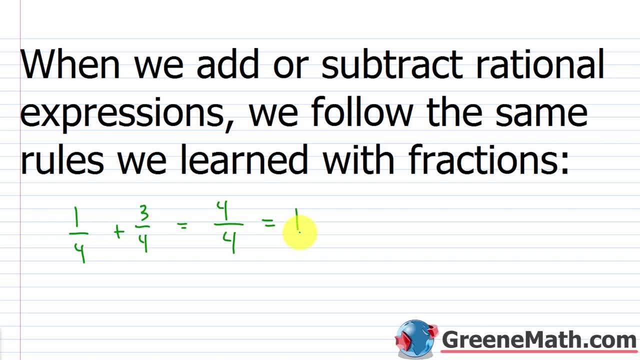 Now what you need to do is subtract, because if you don't know this much, a lot of these words take effort to keys in that statement and query them. So what you need to do is you need to use stupid computers like LCD And then you have to write your fractions as equivalent fractions where the LCD is the. 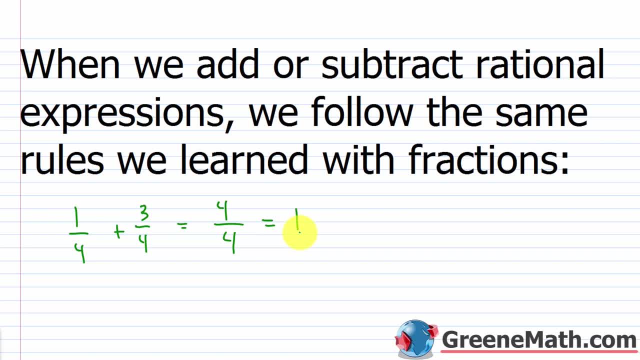 denominator And then you can proceed with your addition or subtraction. So if we thought about something like, let's say, five sixths plus let's say two thirds, just to make it really easy, We know the LCD would be six right, Or hopefully you know that. So I would take five, sixths and I 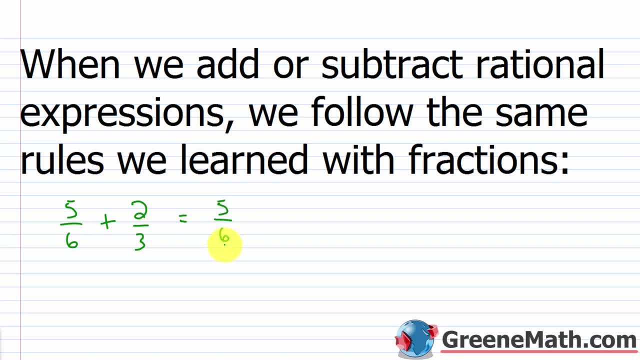 would leave it unchanged, because the denominator is already the same as the LCD For two thirds. I would perform a little trick. I would multiply it top and bottom by the number two. Two over two is the same thing as one. If I multiply by one, I'm not changing something's value. So if I do, 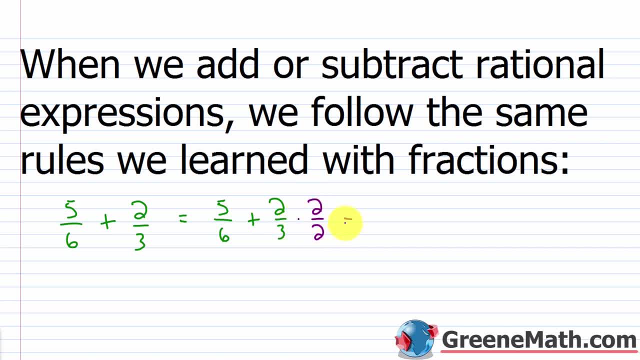 two times two, that's four, And it would be over three times two, which is six. So we can say this is five sixths plus four sixths. And now I can do my addition. My denominator is the same, It's a six. Five plus four is nine, So I end up with nine sixths. 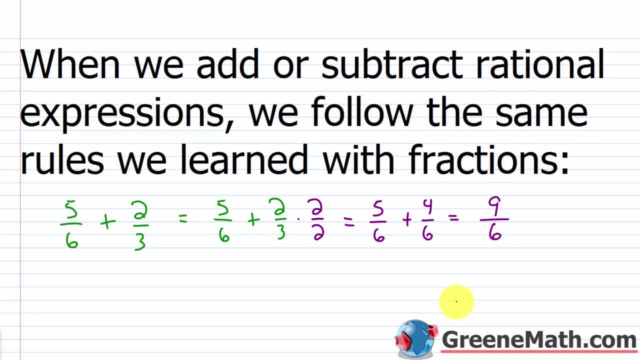 which, of course, we can reduce. Nine and six share a common factor of three. So if I cancel a factor of three here, this would be three. If I cancel a factor of three here, this would be two. So we end up with an answer of three halves. So those are your two scenarios when working with fractions. 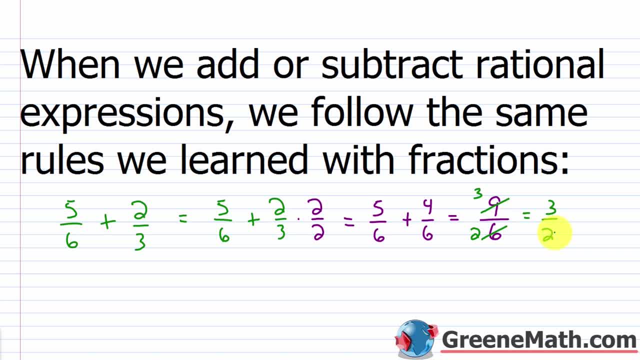 And it's the same exact thing you're going to come across with rational expressions. It's just much more tedious because you're working with variables. the variables have powers. There's all kinds of things that are going on, All right. So let's start out with some real easy ones, just to kind of get our brain going. 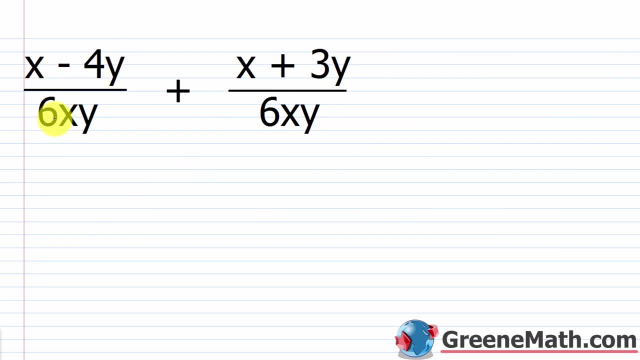 So let's suppose we see x minus four y over six xy plus x plus three y over six xy. So your denominator is the same. You have six xy and six xy, Just like when we work with fractions. again, if the denominator is the same, keep the denominator the same. So for the answer. 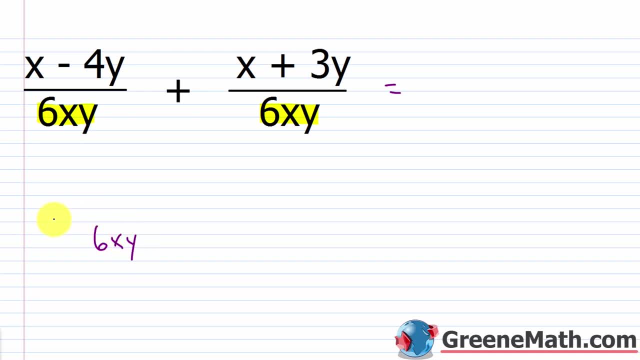 I'm just going to keep six xy in the denominator and I'm just going to add the numerators, So I would have x minus four y It's addition. so I'm just going to put plus and then write this: x plus three y. I'll make this a little longer. 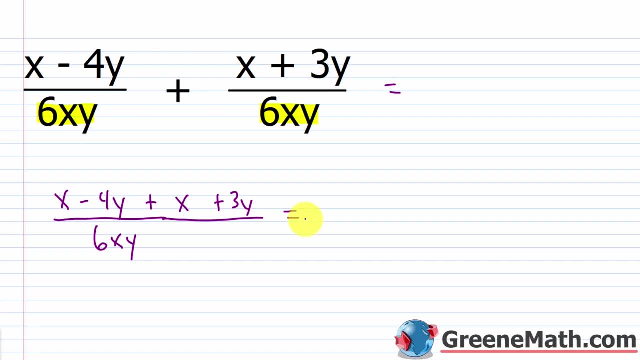 So what would this be equal to? Well, essentially I'm just going to combine like terms: X plus x is what That's, just two x And then negative four y plus three y would be negative y, or just put minus y. And this is over that common denominator of six xy. Now the last. 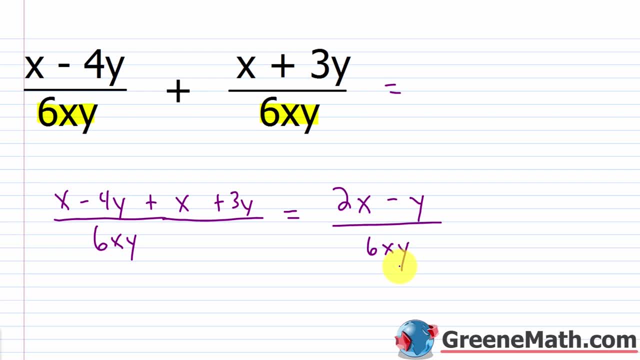 thing you always want to do. you want to see. can I simplify this further? Usually, what you would do is just try to factor everything Now with two x minus y. I can't really pull anything out. If I had something, I'd pull out like, let's say I had a two here. Well, I could pull a two out. 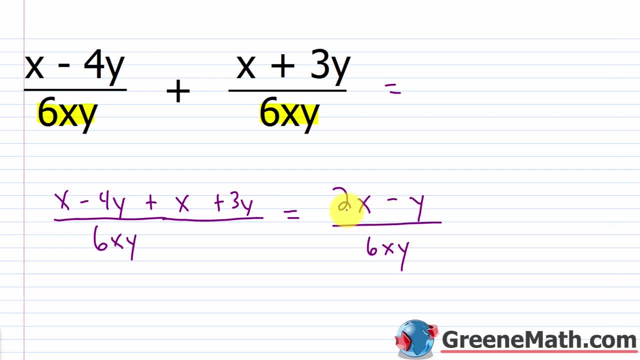 and I could cancel that with the six. But that's not the scenario I have. I have two x minus y over six xy. Nothing I can do to simplify further. So this is our answer right here. All right, let's take a look at another easy one. 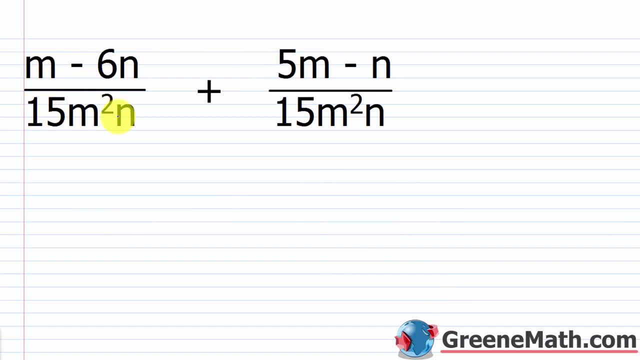 Suppose we have m minus six n over 15 m squared n plus five. m minus n over 15 m squared n. So again the same denominator. So if I have a common denominator already, all I need to do it's very, very simple: I'm just going to add the numerators, So I would have m minus. 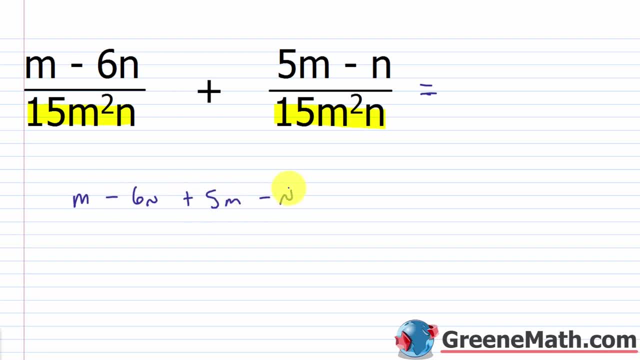 six n plus five m minus n, over that common denominator of 15 m squared n. So I'm just going to combine like terms in the numerator. So m plus five m is six m, And then negative six n minus n is negative seven n, And this is over again, 15 m squared n. So is there anything? I 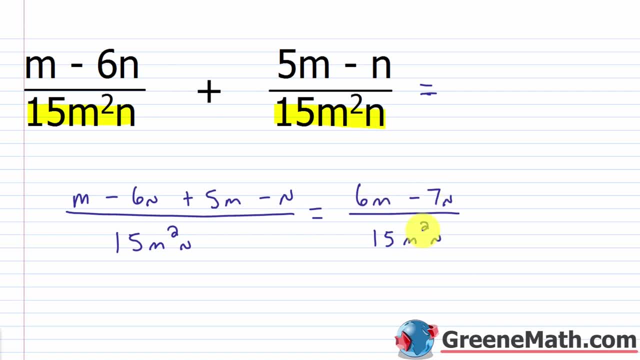 can factor from the numerator here that I could cancel with the denominator? The answer to that is no. You have six and you have seven Number-wise, no Variable-wise. I have an m and then an n, So nothing I can really pull out. So if I had a common denominator I could just 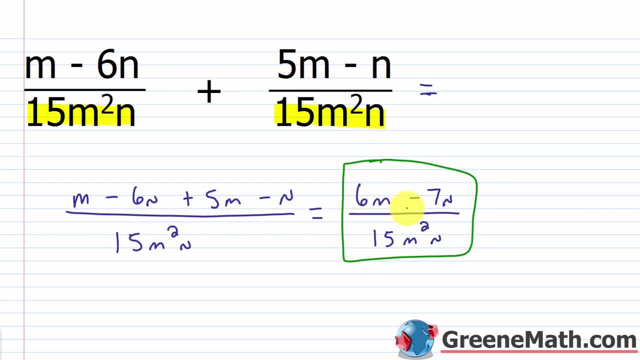 this is going to be your final answer here: 6m minus 7n, over 15m squared n. All right, so let's look at one final easy one, and then we'll look at some scenarios where we don't have a common 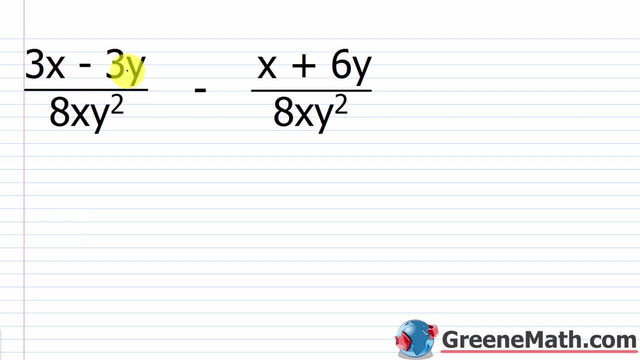 denominator given to us. So we have 3x minus 3y over 8xy squared, minus x plus 6y over 8xy squared. So I'm looking at this and again I notice that I have this common denominator of 8xy squared. 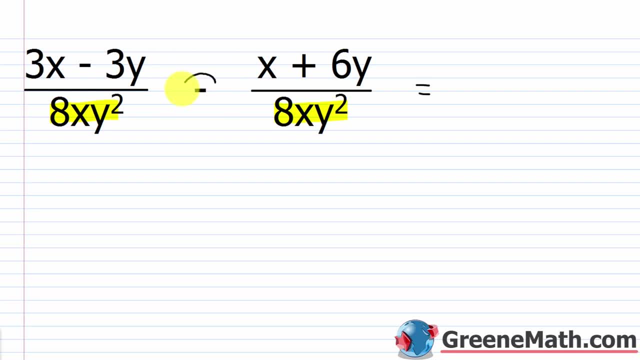 So that just stays the same. I have subtraction here, So this is where you got to be real careful. I am subtracting this whole thing away. So remember, if I'm subtracting something away, I can add the opposite of it. So for the numerator, I have 3x minus 3y. Then what I'm 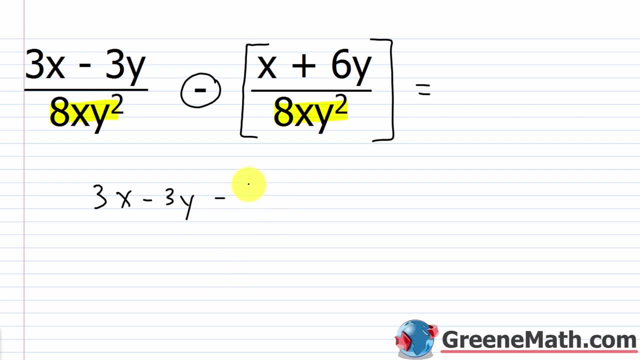 going to do is I'm going to put minus, okay, minus, and I'm going to put inside of parentheses this x plus 3y Plus 6y. That's going to remind me to distribute that negative to each term, and I'm changing the sign of each term. I'm going to add the opposite of it. 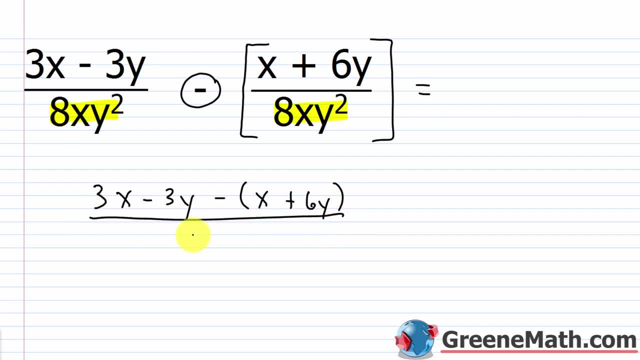 And this is over. We have that common denominator of 8xy squared. All right, so let's go ahead and work this out. We have 3x minus 3y. I'm going to distribute this to each term, So I can think about this as having plus a little negative 1 here, negative 1 times x. 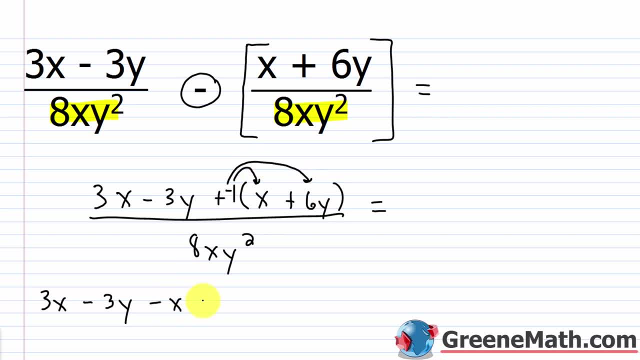 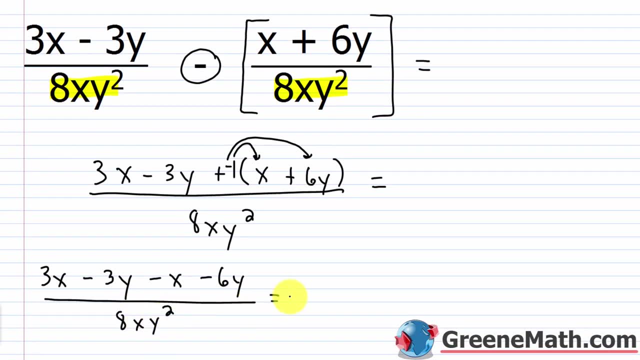 is minus x, And then negative 1 times 6y is minus 6y And this is over. You have 8xy squared. All right, scroll down and get a little room going, All right. so the next thing I'm looking. 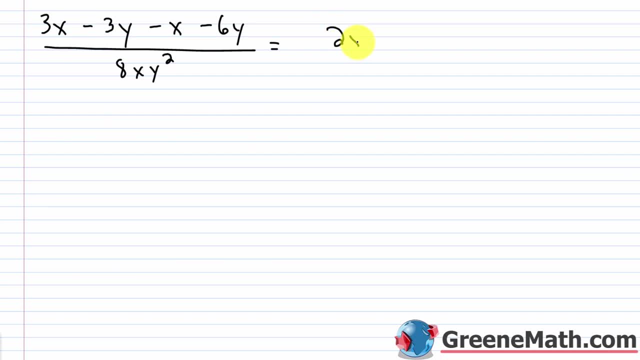 at is: I have 3x minus x, That's going to give me 2x. Then I have negative 3y minus 6y, That's going to give me negative 9y, And this is over that common denominator of 8xy squared. 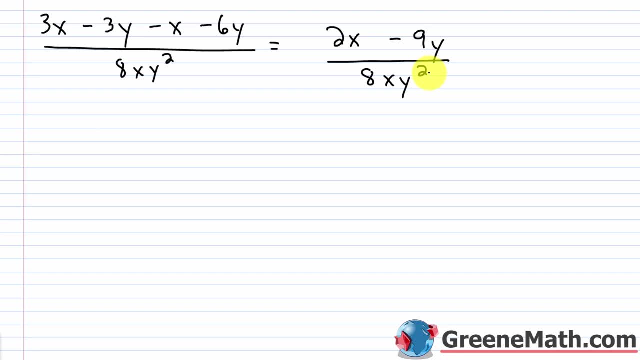 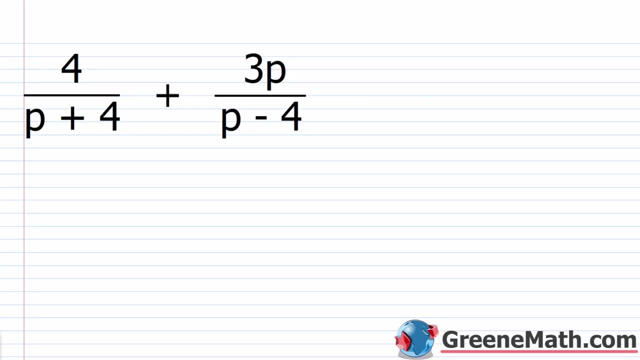 So nothing I can do to simplify any further. I just report my answer as 2x minus 9y over 8xy squared. All right, so let's look at one where there's not a common denominator. We'll start out with. 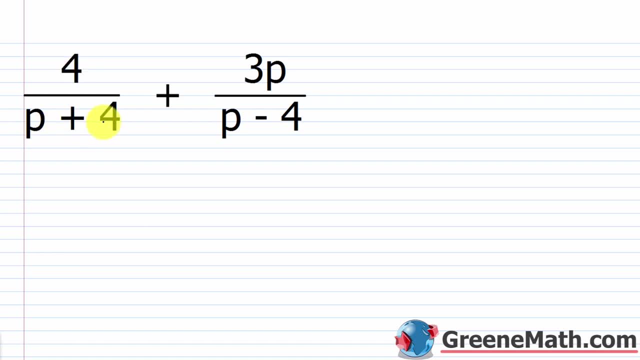 something pretty simple: We have 4 over p plus 4, plus 3p over p minus 4.. So before we even do this, let's just think about two fractions. for a second, Let's say, I had something like 1 third plus. 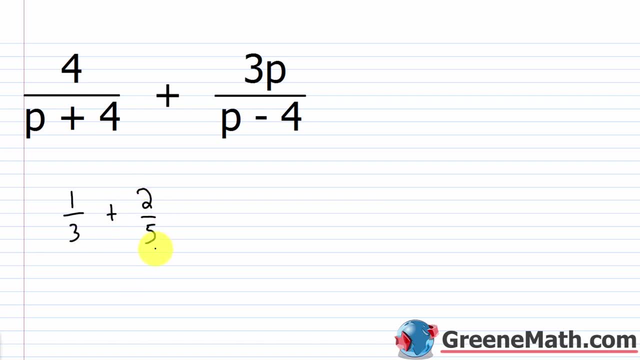 I don't know. let's say 2.. So you get the LCD. What do I do? I take the denominators and I factor them. Now, 3 and 5 are each prime number, So there's not really anything I can do to factor them. They're just 3 times 1, or 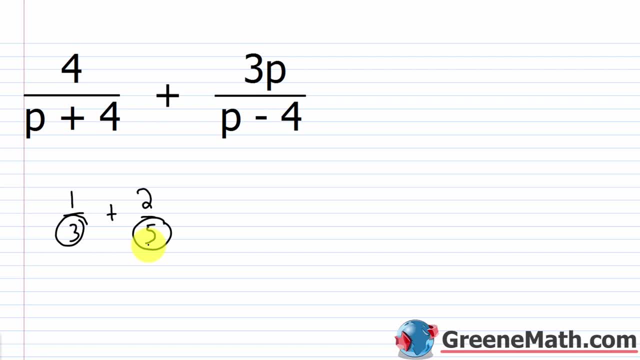 5 times 1.. So what I want to do when I build my LCD, my LCD, that's what It's the least common multiple of these two numbers, So of 3 and 5.. And so to do that when I have my factorization. 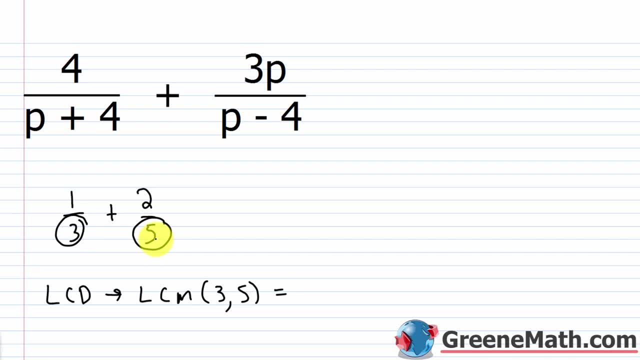 I list Each prime factor. The only exception is when I have a duplicate prime factor. So if I have a prime factor that occurs in each prime factorization, I go with the largest number of repeats. Now in this case I just have a 3 and a 5.. So I would put 3 times 5 and that would give. 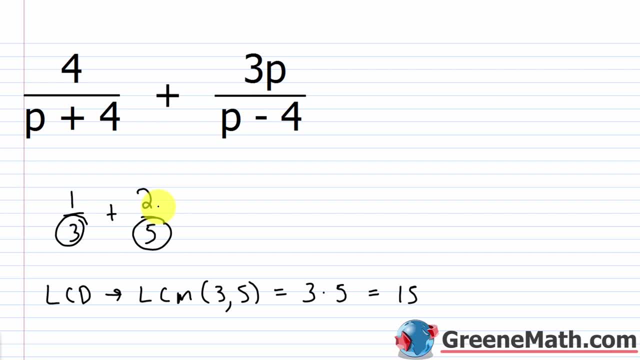 me 15.. So I would convert each of these into an equivalent fraction where 15 is the denominator, and then I could do my addition. So hopefully you remember how to do that. I know for some of you it's been quite a lot of time. So I'm going to do that. So I'm going to do that. So I'm going to. 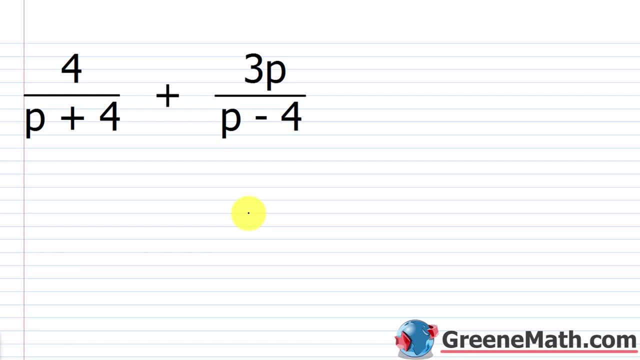 do that, But it's going to be the same process here. I look at my denominators, So I have P plus 4 and I have P minus 4.. So the question is: can I factor P plus 4? No, I cannot. Can I factor P minus? 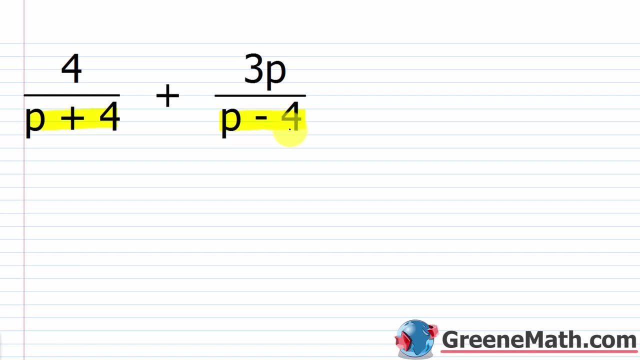 4?? No, I cannot. So, just like when I had a denominator of 3 and a denominator of 5 and I couldn't factor them, I just multiplied the two together. I'm going to do the same thing here. So the LCD is going to be what It's going to be- the same thing. So I'm going to do the same thing here. 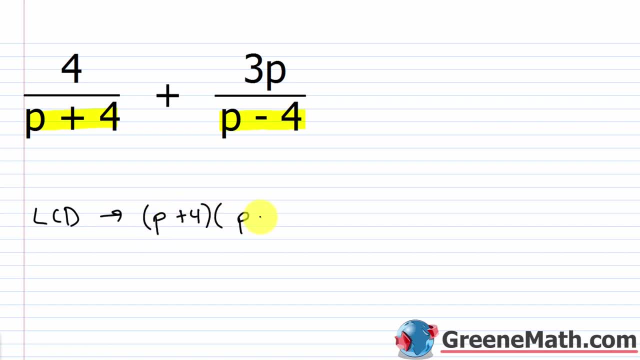 It's going to be P plus 4 multiplied by P minus 4.. And generally we want to leave this in factored form. I know you could use FOIL here and kind of write it in a different format, but we want to. 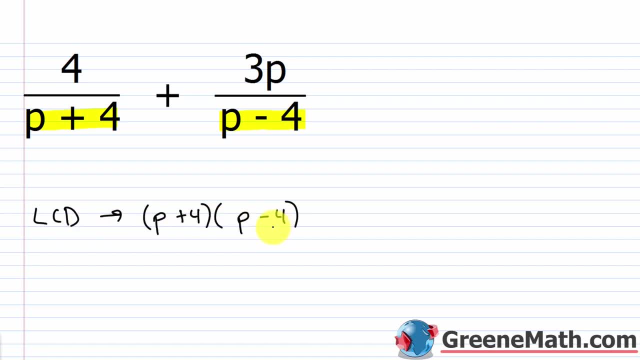 leave it like this, All right. So if this is the LCD- and I have, let me kind of just drag this up here so it's out of the way- So if I put equals here, I'm going to have 4 over P plus 4.. Now the 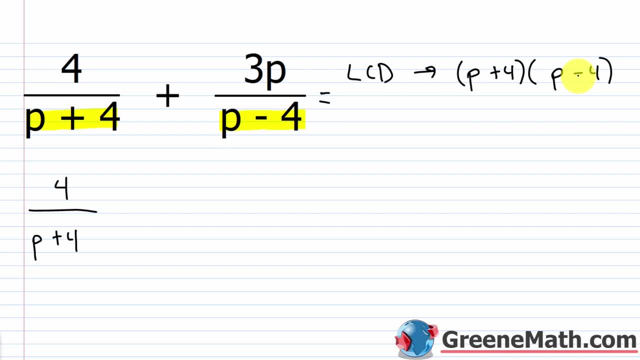 LCD is what It's: P plus 4 multiplied by P minus 4.. So I'm going to do the same thing here, So I'm going to have 4 over that quantity times P minus 4.. So in order to have a denominator of P plus 4, 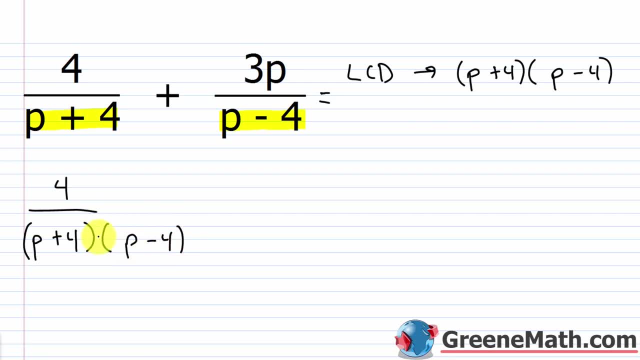 times P minus 4, I've got to multiply the denominator by P minus 4 and also the numerator by P minus 4.. Make sure you're using parentheses here, because again, this is the quantity P minus 4.. Okay, Don't make that mistake of saying, okay, I've got 4P minus 4 like that. That's wrong, Okay. 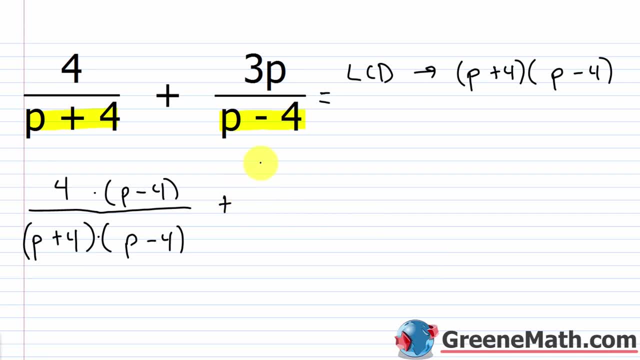 You don't want to do that, Then you're going to have plus. So next you see, you have 3P over, you have P minus 4.. And what am I missing here? Well, I'm missing the P plus 4.. So let's multiply the top and the bottom by the quantity P plus 4.. 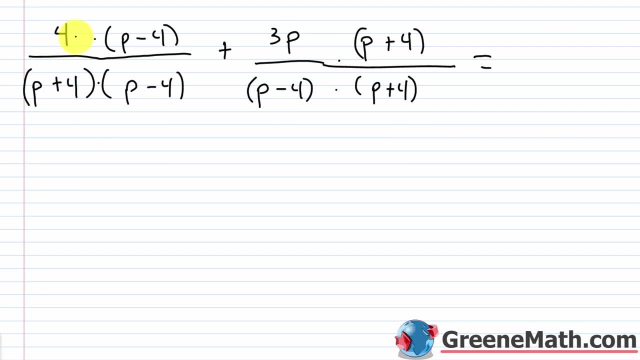 And let's scroll down and get a little room going. So if I do 4 times the quantity P minus 4, I'd have 4P minus 16. Then plus you have 3P times P. That's 3P squared. 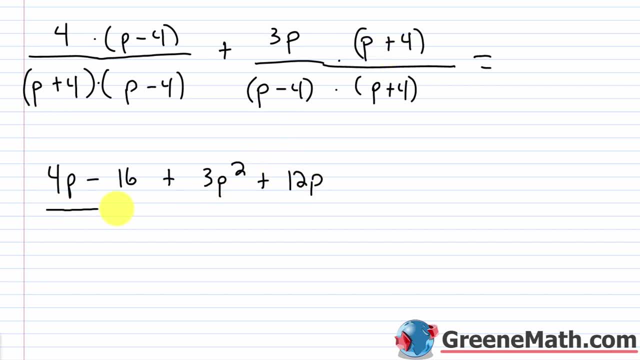 Then 3P times 4 is plus 12P And this is over. You've got P plus 4, that quantity times P minus 4, that quantity. So if I combine like terms in the numerator you kind of scroll down. 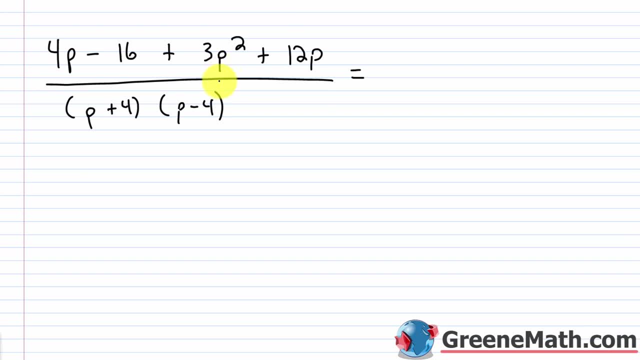 get a little room going, I'm going to start out with 3P squared, Then next I look, I see 4P and 12P. Well, that would combine to give me 16P, And then, lastly, I'd have minus 16.. So then, 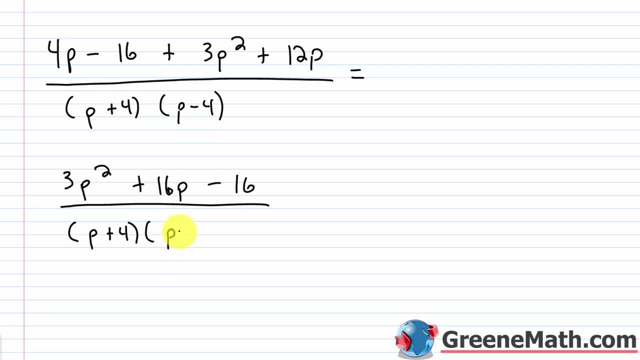 this is over. We have P plus 4 times P minus 4.. So I'm not done, because with these I want to see if I can factor something. I have left this in factored form to see if I can cancel, So let's. 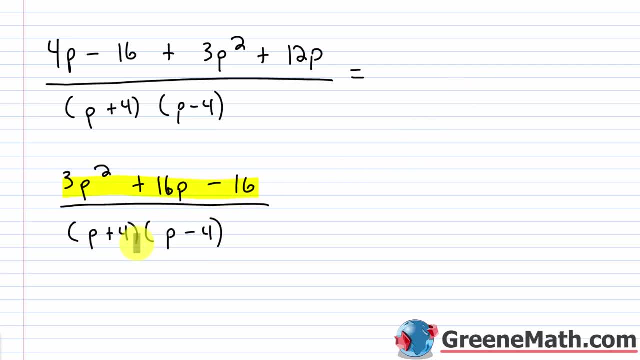 try to factor this right here into the product of two binomials And let's see what we get. We're trying to see if we can cancel anything with the denominator. So give me two integers whose product is 3 times negative 16 or negative 48.. 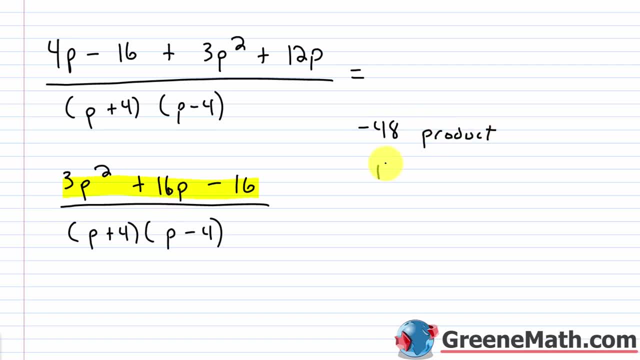 This is my product I'm looking for, And we want a sum of 16.. So we know we need one positive and one negative. So let's think about the factors of just positive 48. Forget about the fact that it's negative. So for 48, you've got what You've got. 1 and 48. Those are obviously too far apart. 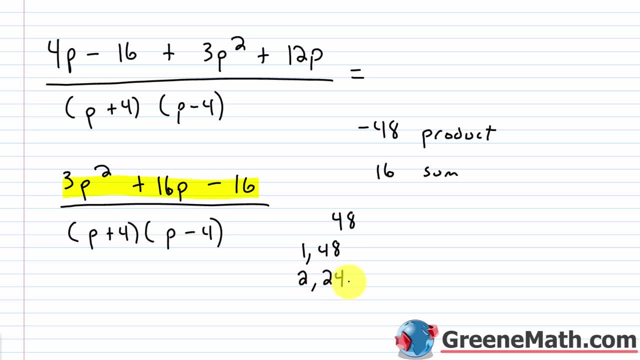 You've got 2 and 24.. Those would never work. It is divisible by 3.. It's 3 times 16, but those won't work. Now you could also do 4 times 16.. You could also do 4 times 16.. You could also do. 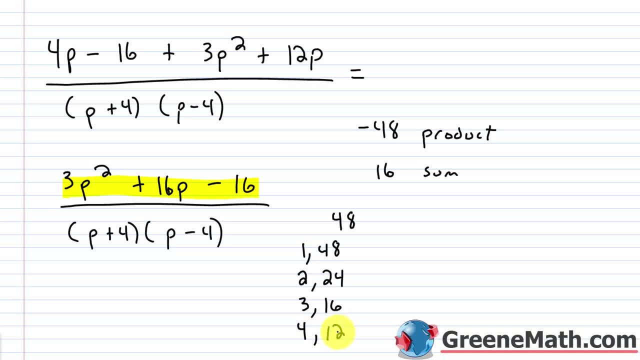 4 and 12.. Now it seems like 4 and 12 would work because you've got a positive 16 there. So you could say: OK, well, 4 plus 12 is 16, but you can't make the sign work with the product If I made one. 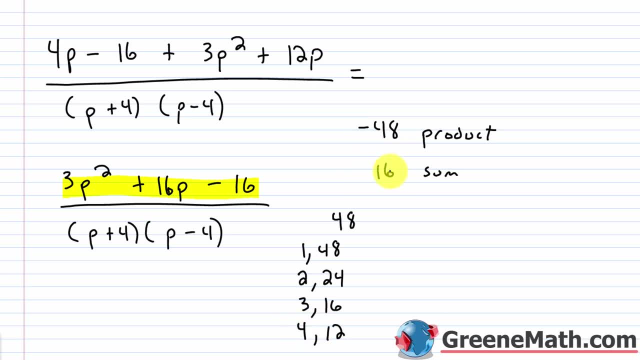 of those positive and one of those negative, you will not get to that sum. So then the next thing we try: it's not divisible by 5., It is divisible by 6. It's 6 and 8. So 6 and 8. But that won't. 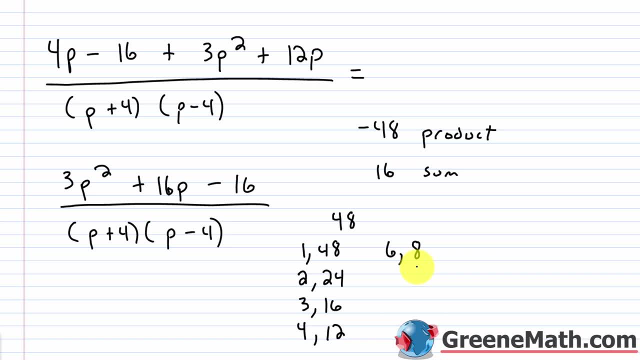 work. So after 6 and 8, we don't have any more factors. So I would say this polynomial is prime. So let me erase this And I will say that this is prime. And because this is prime, there's nothing else I can do to simplify it. And so this is my answer: 3p squared plus 16p. 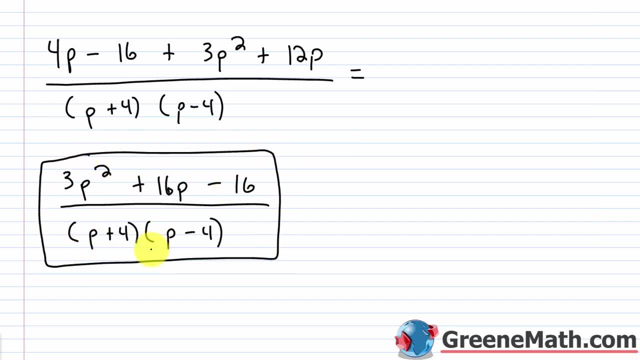 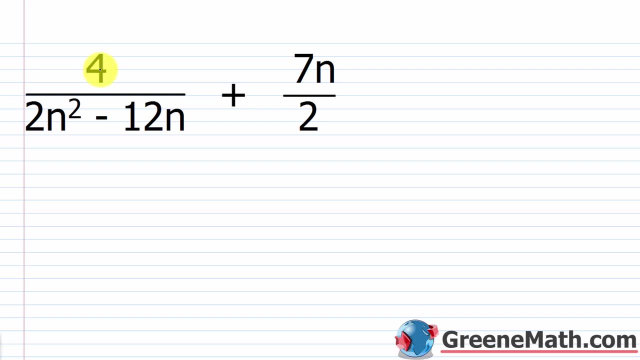 minus 16 over the quantity p plus 4 times the quantity p minus 4.. All right, let's take a look at another kind of easy one. So we have 4 over 2n squared minus 12n, plus 7n over 2n squared minus. 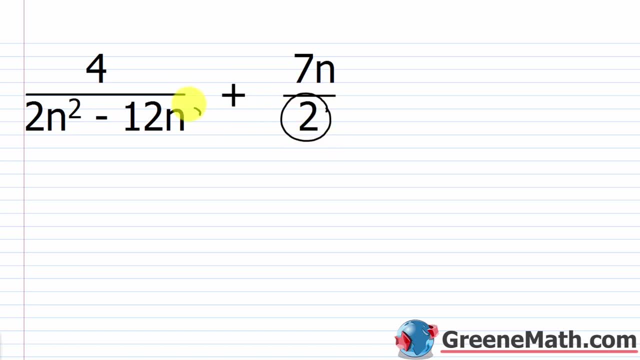 2.. So I've got a denominator that's just a 2. And I've got a denominator that's a 2n squared minus 12n. So I can't really factor 2.. It's a prime number, It's just 2.. If I factored this, what? 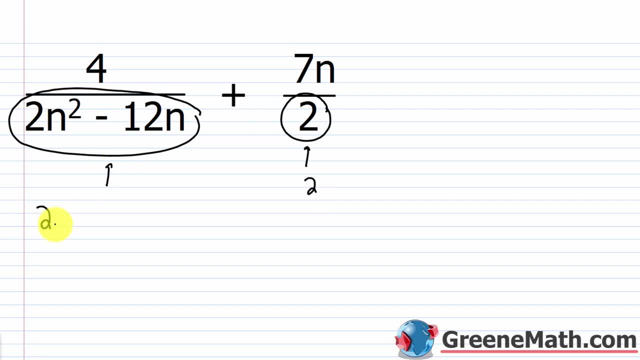 could I do? Well, I could pull out a 2n, I could pull out a 2n, And then I would multiply that by the quantity n minus 6.. So, because this already has a 2 and this has a 2, when I think about my 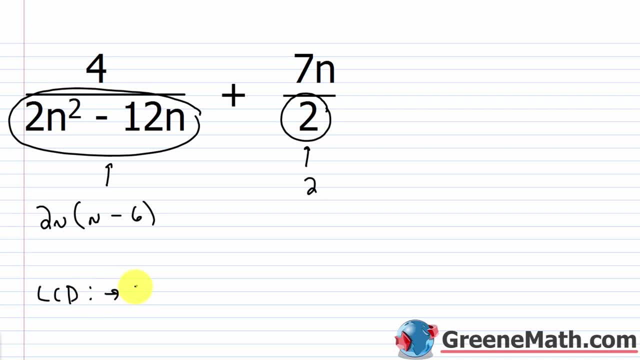 LCD, it would have a 2. And then it would have the rest of this times n times the quantity n minus 6.. So this guy right here already has all that. All I need to do is change this rational expression here. So let me again move this up and out of the way. We'll say this equals- I'll. 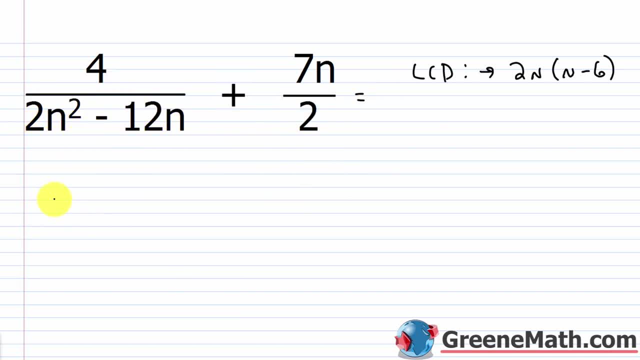 erase this real fast. So for the first guy, I'm just going to write 4 over And I'm going to write this in factored form. So 2n times the quantity n minus 6. Then, plus For this guy, I have 7n over 2. And I'm multiplying by what I'm missing. So I'm missing an n And 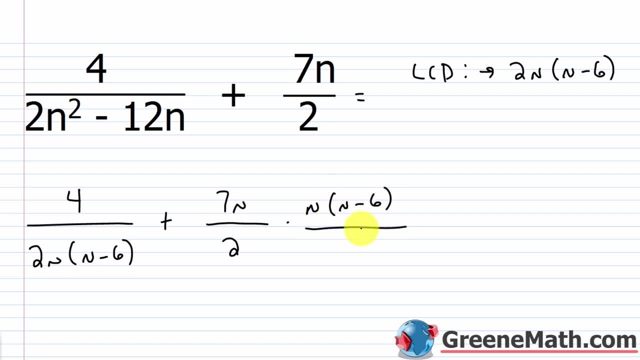 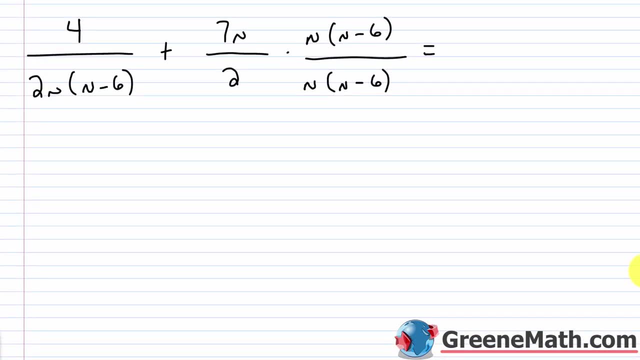 I'm missing the quantity n minus 6.. All right, So let me put equals And we'll just scroll down and get a little room going. We'll have 4 plus. We're multiplying three of these guys together. We're multiplying three of these guys together. We're multiplying three of these guys. 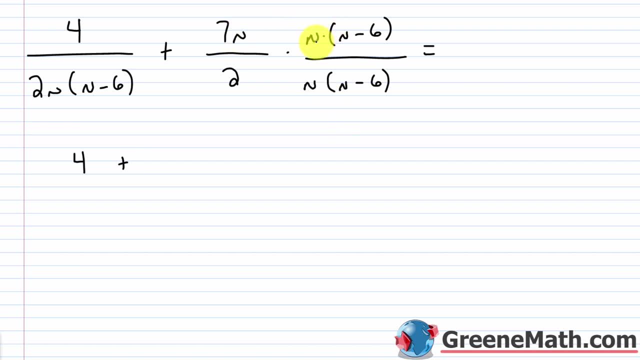 together, So the order isn't going to matter. I could do 7n times n first. That would give me 7n squared. So let me put 7n squared here And then times the quantity n minus 6. And let me just do. 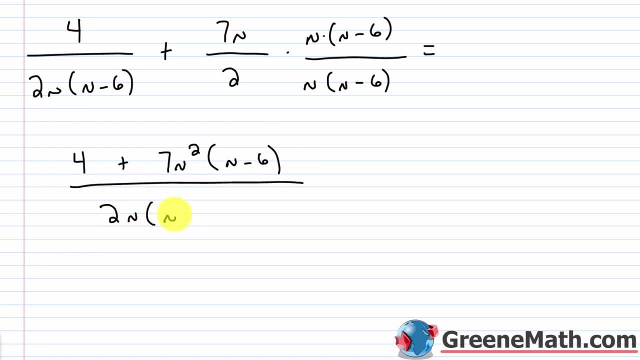 this down here. The denominator we know will be 2n times the quantity n minus 6.. All right, So we'll continue. We have 4 plus. You have 7n squared times n, That's 7n cubed And then 7n. 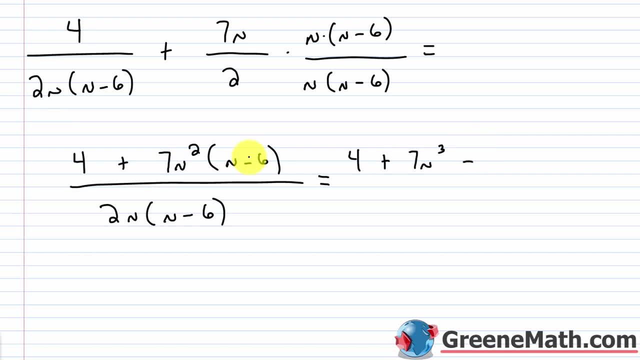 squared times negative. 6 would be negative. 7 times 6 is 42.. And then you have 7n squared times the quantity n minus 6. And your n squared would come along for the ride. And this is over We have. 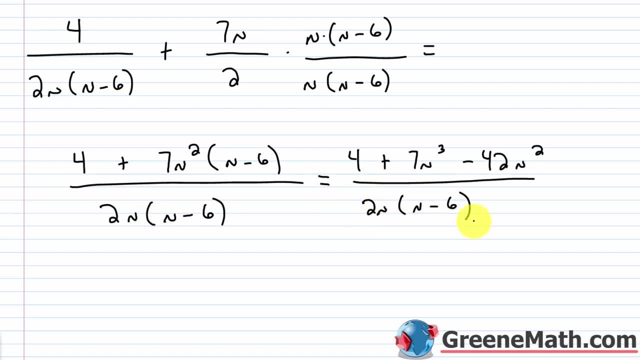 2n times the quantity n minus 6.. So this isn't going to be something we can factor in the numerator, But I can reorder it. Put that polynomial in standard form. We'll write 7n cubed minus 42n squared. Let me kind of make that a little better. And then, lastly, plus 4.. 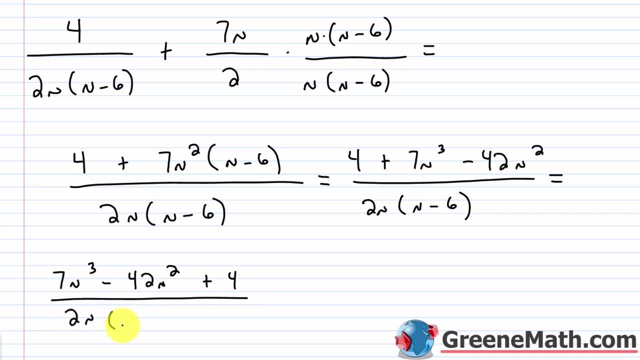 And then all over 2n times the quantity n minus 6.. Again, I leave this in factor form in the denominator, just to show that nothing is going to cancel. Let's look at one that's a little bit more tedious. So we have 7 over, We have 2n cubed. 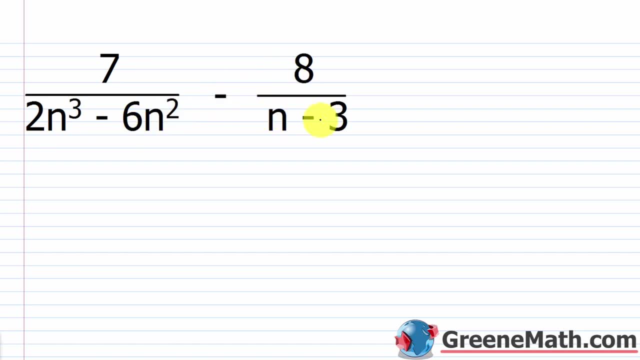 minus 6n squared, Then we have minus 8 over n, minus 3.. So remember, I have this minus here. So I've got to be very, very careful What I can do. I can put that this is plus And then I can make. 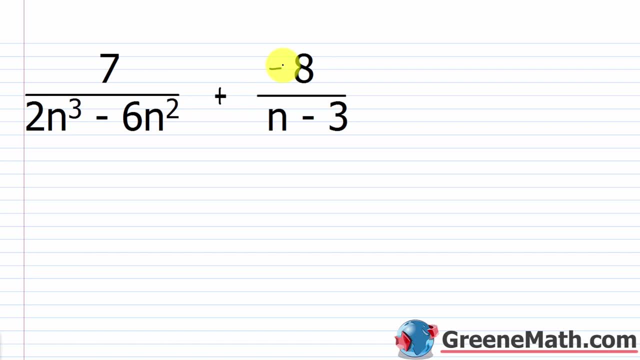 this a negative 8. If I put plus and then I change something to its opposite meaning, I multiply it by negative 1. I'm good to go. That's preferable to what we normally do, Because students will get confused. So once I've rewritten this problem, I think about the denominators. So this is 2n cubed minus 6n. 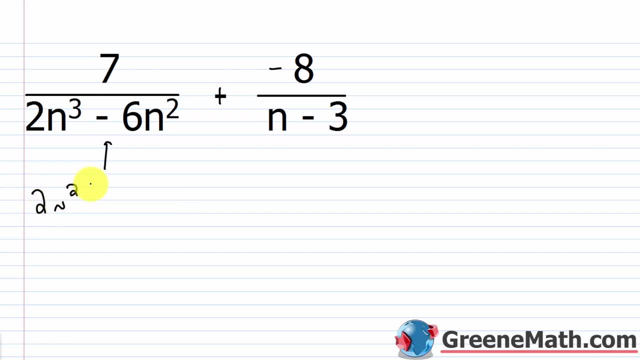 squared, I could factor out a 2n squared And I'd be left with n minus 3.. And then here I just have an n minus 3.. So what's common to both? They each have this n minus 3?. I'm just missing. 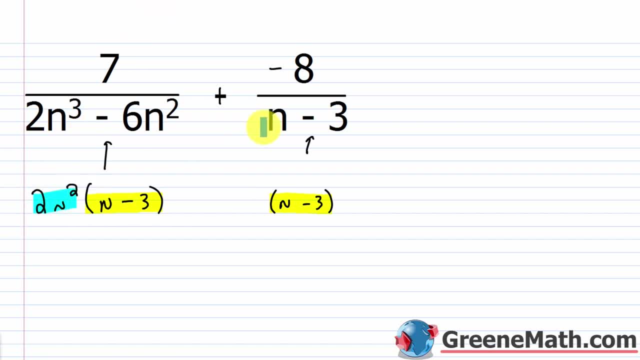 the 2n squared. I'm just missing this 2n squared. So again we come to the scenario where this first guy here is unchanged. We're just going to have 7 over. we have 2n squared times the quantity n minus 3, and that's in. 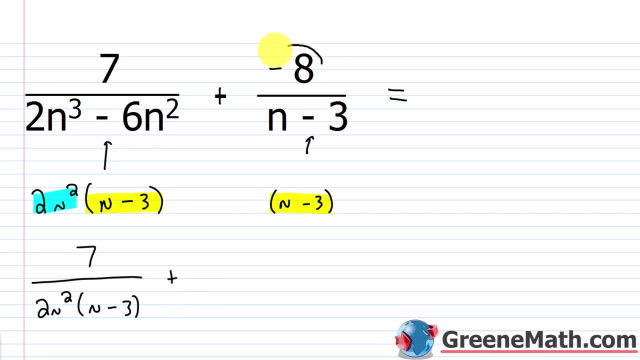 factor form. Then I'm going to put plus. remember I changed this to negative 8, so we'll have negative 8 times. what am I missing here? I'm missing 2n squared, So times 2n squared over. 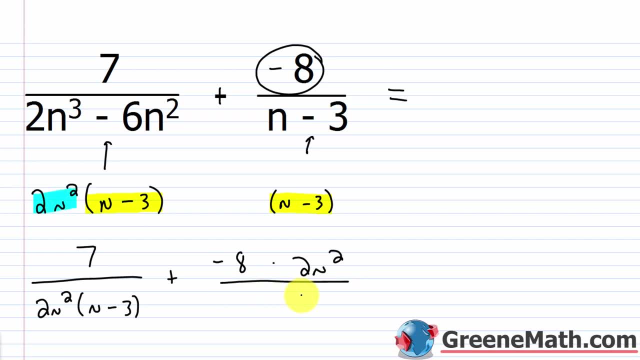 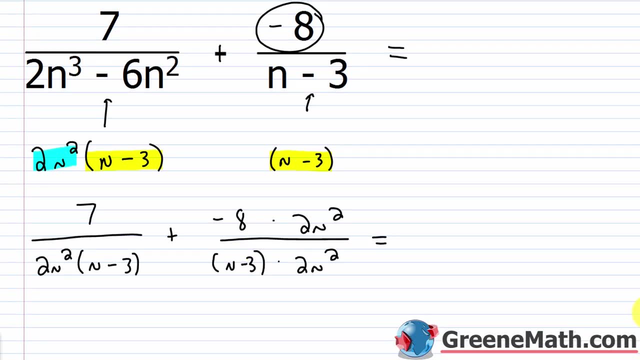 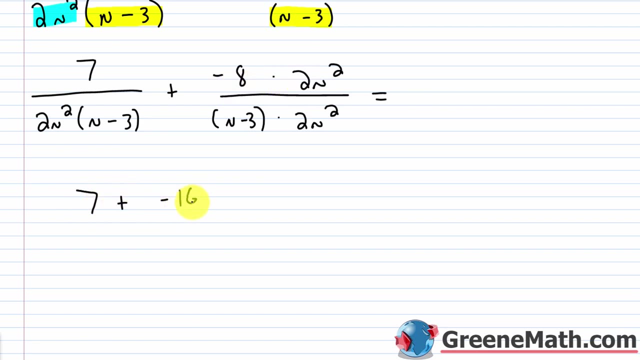 you would have n minus 3 times 2n squared. So I'll put 2n squared over here like this: times that quantity n minus 3.. So now I have a common denominator and so I can just go through now. So I have 7 plus negative 8 times 2n squared is negative 16n squared, and then this is over. 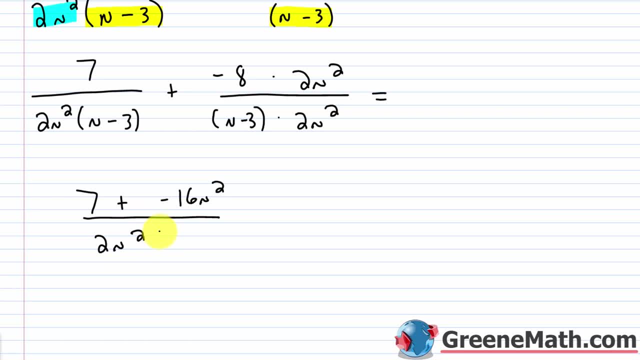 we have 2n squared times the quantity n minus 3.. So let me just reorder the terms and we'll put negative 16n squared over, and then this is over, and then this is over squared plus 7, over 2n squared times the quantity n minus 3.. So not really anything I'm going to be. 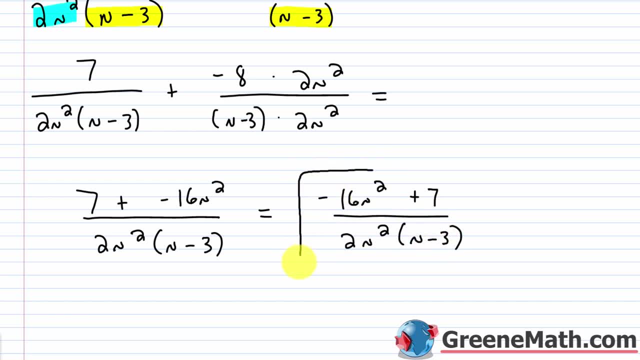 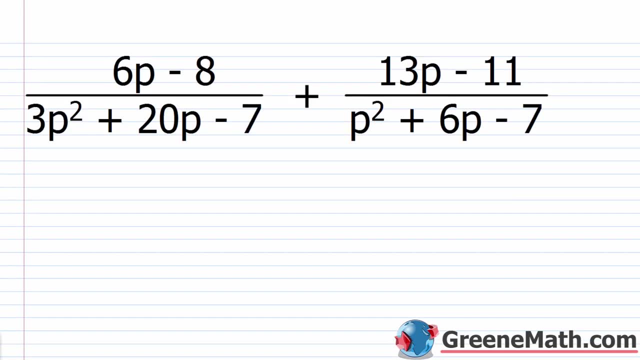 able to do to simplify this any further. So we just leave our answer like this: We have negative 16n squared plus 7 over 2n squared times the quantity n minus 3.. All right, now let's get into one of the more tedious problems, And you'll typically see more of these in Algebra 2 than you. 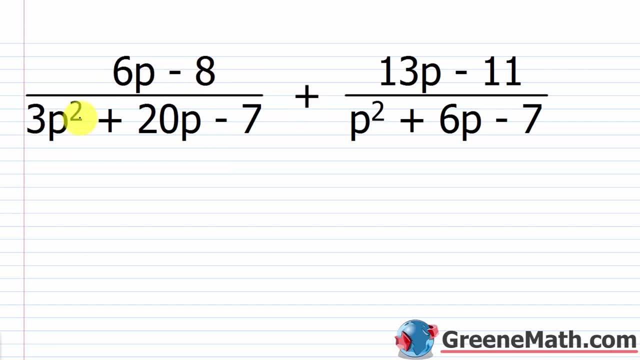 did in Algebra 1. So you have 6p minus 8 over 3p, squared plus 20p minus 7, plus 13p minus 11 over p squared plus 6p minus 7.. So I want to just start by getting a common denominator. So I'm going to. 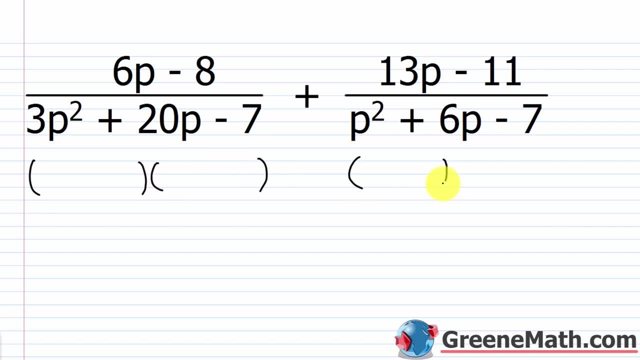 factor this guy right here, And I'm going to factor this guy right here, So I know this one's easier. So let me just start with that. I know this would be p and this would be p: Two integers whose product is negative 7 and whose sum is positive 6.. I could do. 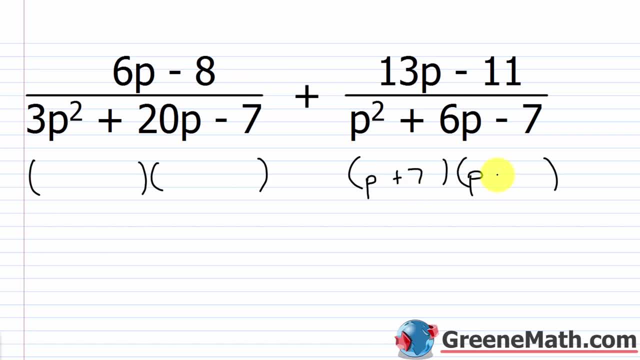 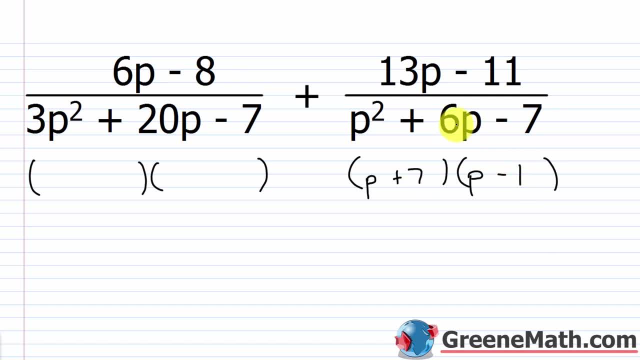 negative 7.. 7 plus negative 1 is positive 6.. So that checks out For this guy right here. I've got a non-1 as my leading coefficient, So it's a little bit more challenging to factor. We can use reverse FOIL. just to get a little practice, Let's go with 3p and p Remember. 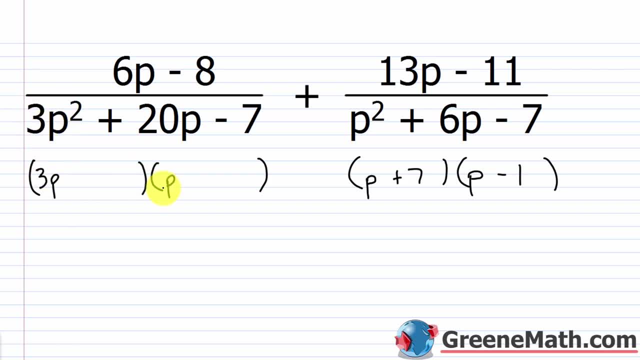 this is a prime number, So I go with that to start. Now I need to work out my outer And my inner to where the sum is 20p and the product is negative 7. Now it's easy, because negative 7, or just 7 in general, is a prime number. So really the only possibilities are: 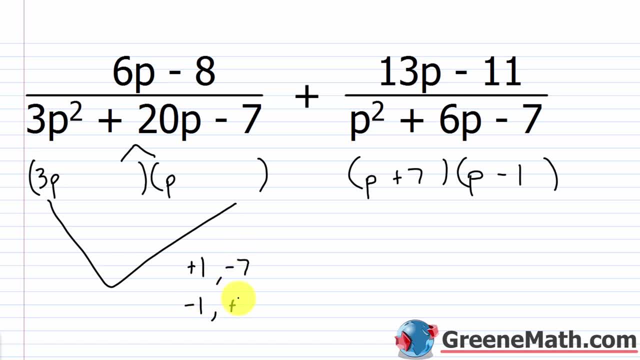 positive 1 and negative 7, or negative 1 and positive 7.. So I can try different combinations. I could say: okay, if I had positive 1 and negative 7, like this. what would that give me? Well, the outer, just think about the numbers. 3 times negative 7,. 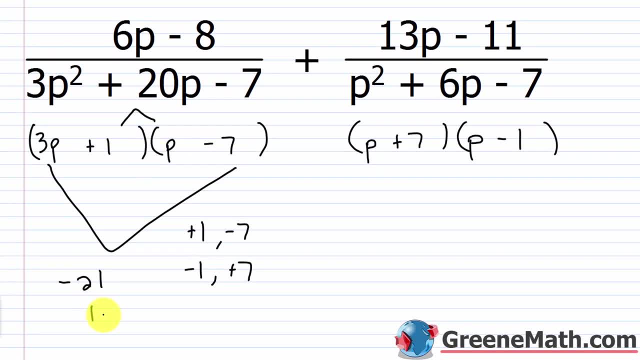 is negative 21.. The inner 1 times 1 will be 1.. So if I sum those, I would end up with a negative 20.. Well, I want a positive 20.. So all I have to do is just change the signs around. 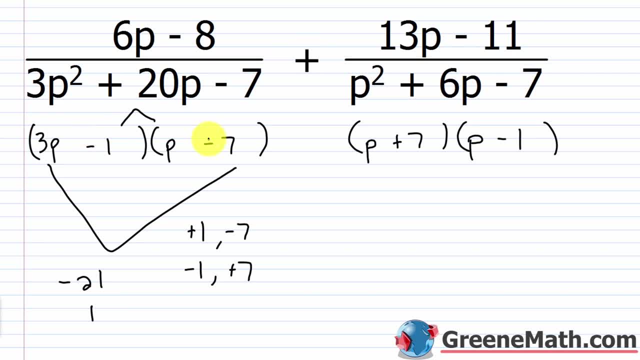 Everything is in the right position. So if I make this negative and this positive, I'm going to be good to go, Because my outer would be 21p. 3p times 7 would be 21p. My inner would be negative p. Those would sum to be 20p. All right, So I've got my factorizations. 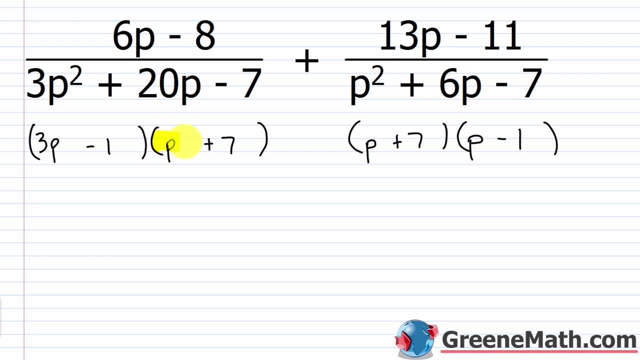 going. What do they share? Well, they each share P plus 7. So that's already there. All I need to do to think about the LCD again. everything gets listed, but what they share, or what's common to both, just gets listed once. 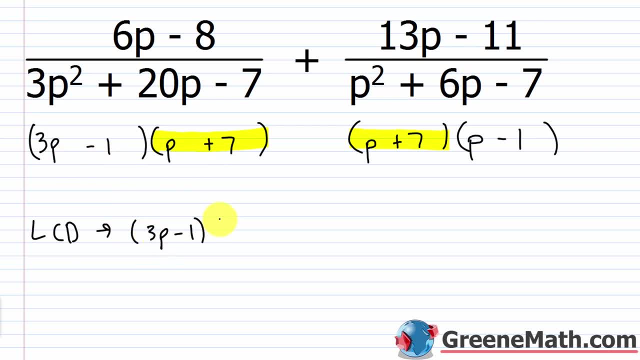 So I would put 3P minus 1, then times P plus 7, and I've got a P plus 7 here and a P plus 7 here, so it only goes in once You go with the largest number of repeats between any factorization. 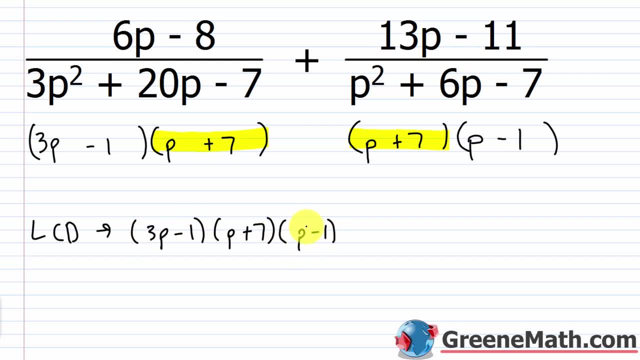 Then I've got a P minus 1.. So that's my LCD. So in other words, for this first one here I am missing the P minus 1.. So I'm going to multiply 6P minus 8 times the quantity P minus 1.. 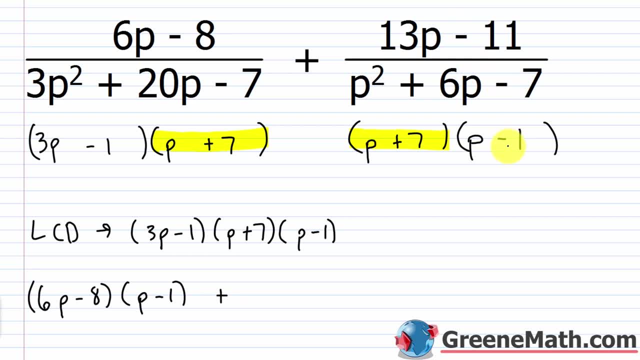 Then, plus over here, what am I missing? Well, I have P plus 7, I have P minus 1, I'm missing 3P minus 1.. So I'm going to multiply 13P minus 1.. Plus 11 times again what I'm missing, which is this: 3P minus 1.. 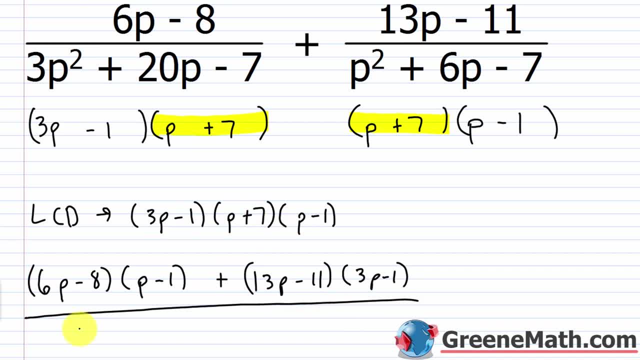 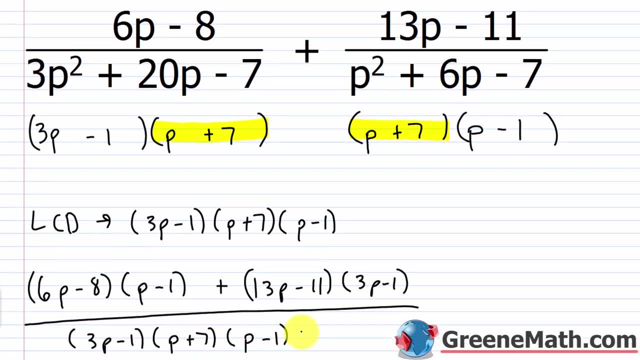 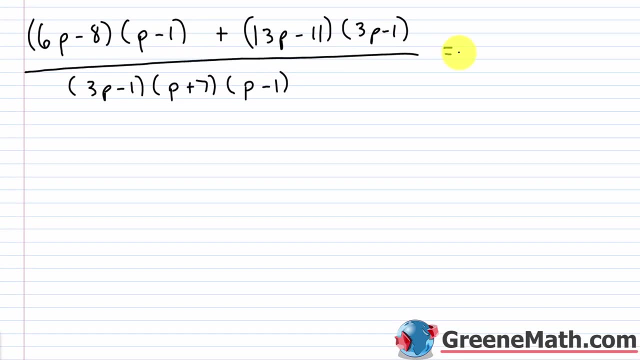 Then for the denominator. we already know that's going to be the LCD. So that's 3P minus 1 times P plus 7 times P minus 1.. And again these can get quite tedious very, very quickly. So let's go ahead and use FOIL here. 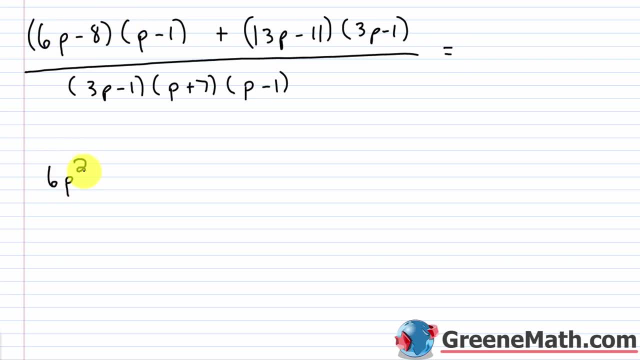 6P times P is 6P squared. The outer 6P times negative 1 would be 4P. It would be negative 6P. The inner negative 8 times P would be negative 8P. We can go ahead and combine like terms here. 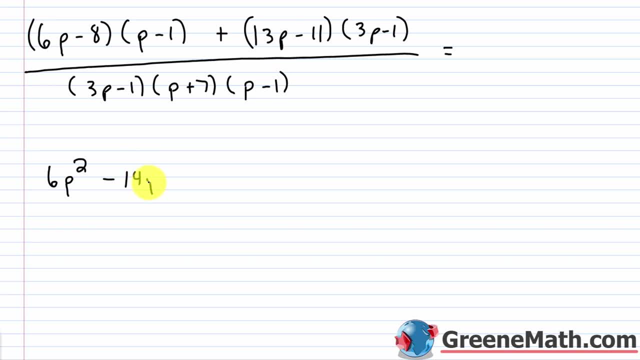 We know that's negative 14P And the negative 8 times negative 1 is positive 8.. Then we have plus Over here: 13P times 3P is 39P squared. The outer 13P times negative 1 is going to be negative 13P. 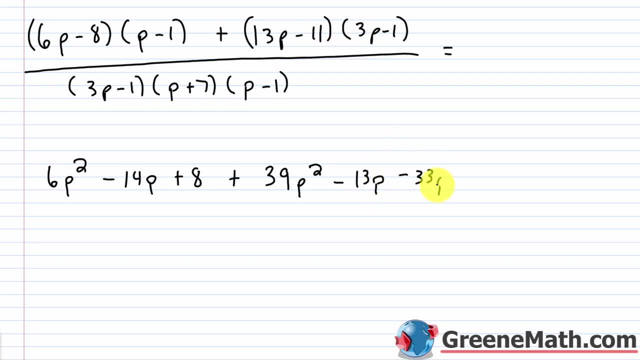 The inner negative 11 times 3P is minus 33P. And then the last negative 11 times negative 1 is positive 11.. All right, So what can we do to combine like terms here? Let me write this over: that common denominator of 3P minus 1 times P plus 7 times P minus, 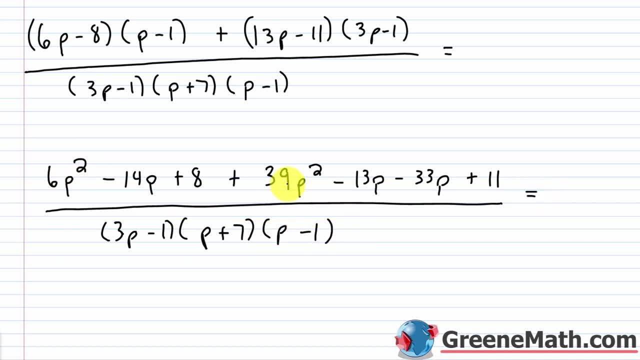 1. So I have 6P squared and 39P squared, So that would give me 45P squared. Then next I have negative 14P, I have negative 13P, That's negative 27P, And then minus another 33P, which would be negative 60P. 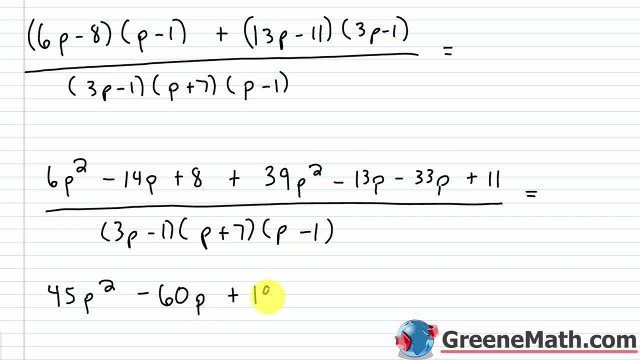 And then, lastly, I have 8 plus 11, which is 19.. So this is all over. We have 3P minus 1 times P plus 7 times P minus 1.. So is this guy in the numerator factorable? 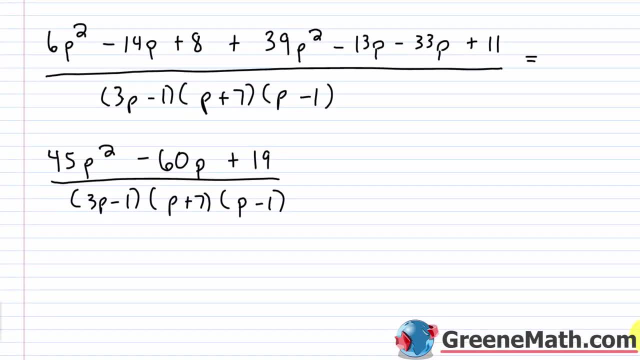 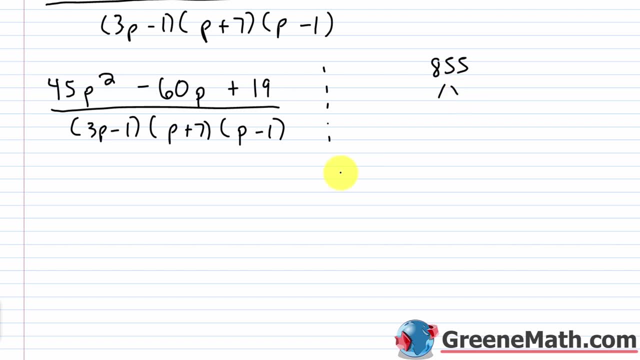 We think about 45 times 19.. We think about 45 times 19.. That's 855.. It's a pretty big number. So I think about 855 as the product I would be looking for for the two integers, but it 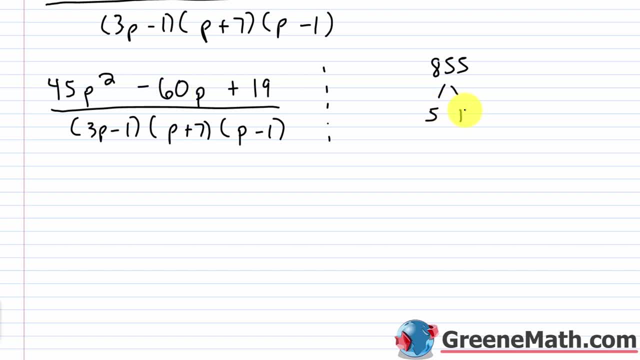 would have to sum to negative 60.. Well, this would be 5 times 171.. Five is prime, 171 is 19,, which is prime times 9.. Nine is 3 times 3.. So not a whole lot of factors for 855.. 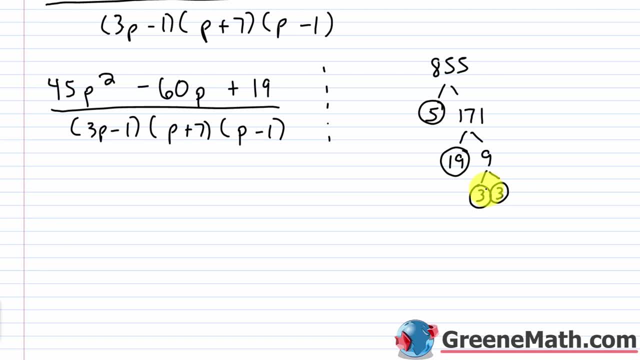 If I played with the signs? let me just think about this for a second: If I played with the signs, could I make it work? The answer to that is no, So let's just quickly go through these factors real quick, so you can see. 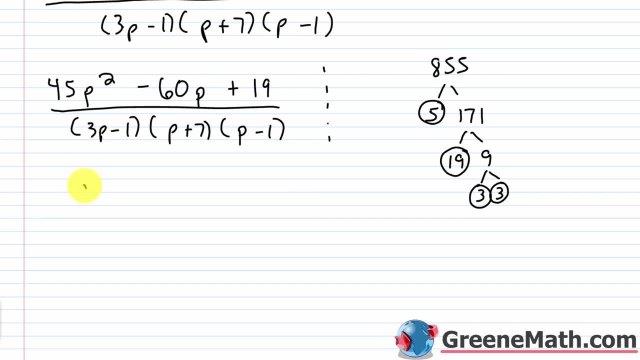 The first thing would be 1 and 855.. We really don't need to list that, but we will anyway. We know those are too far apart, So this will never work, So let me just line that out. The next thing you would come across: just look at your factor tree. 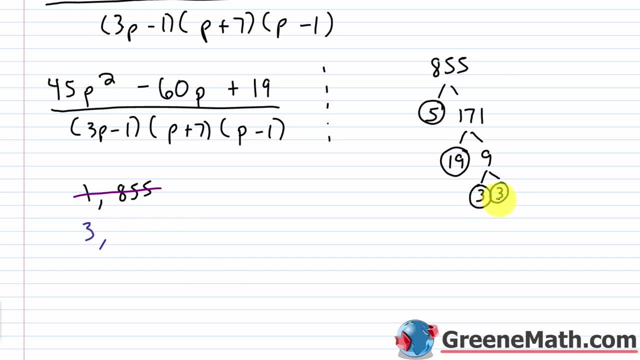 You'd have a 3.. So 3 times what? Well, what's left? 3 times 19 times 5,, which is 215.. So what's left? What's left? 185.. Again, those are way too far apart. 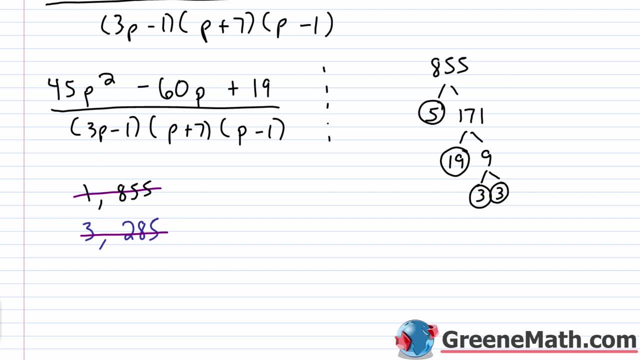 So even playing with the signs, I'd never get anywhere. So the next thing we would come across, we see we have a 5,, so I could put 5, and then what It would be 19 times 3 times 3,, which is 171. 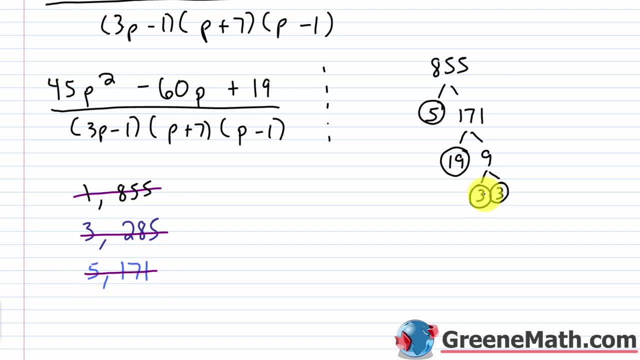 But again I can't play with the signs and make that work. So then I would go to 3 times 3, or 9, times what You'd have, 19 times 5, or 95. But again that's not going to work. 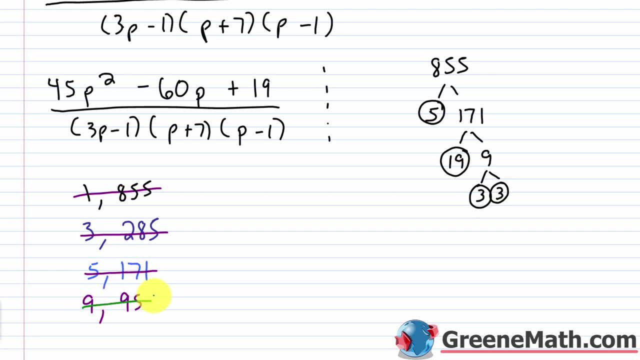 I can't play with the signs and make that get to negative 7. Negative 60. So next I'd think about 5 times 3, or 15.. 15 and what We'd have? 19 times 3, or 57.. 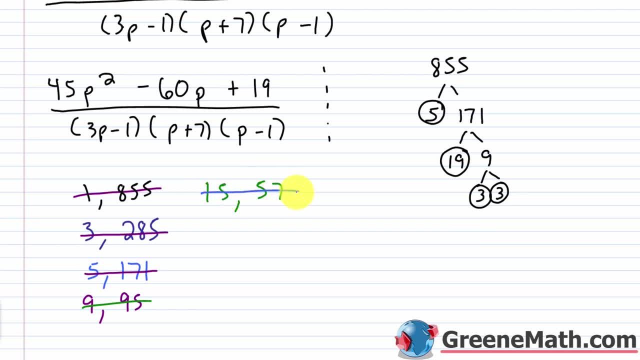 Again, those aren't going to work. so you can line that out. Then the last thing you could try is 19 times 45. So 19 and 45, and those obviously wouldn't work. So I'm out of possibilities here. 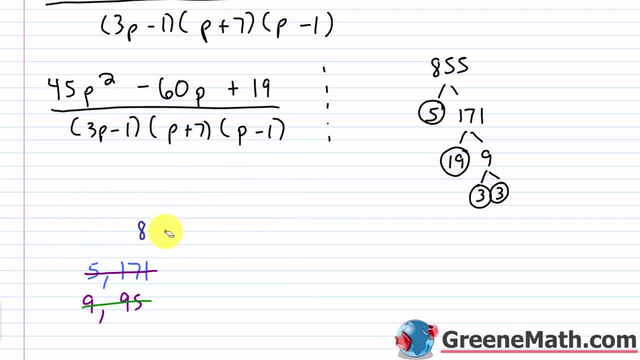 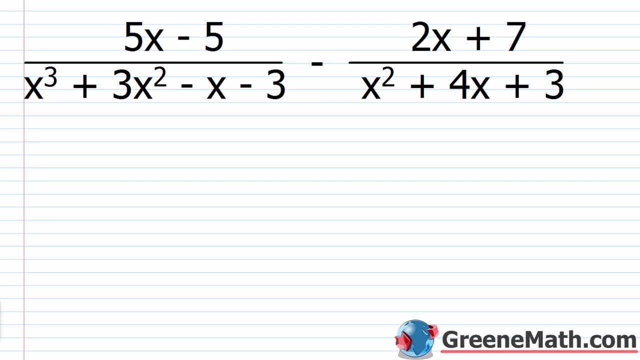 So I can erase this And just declare. 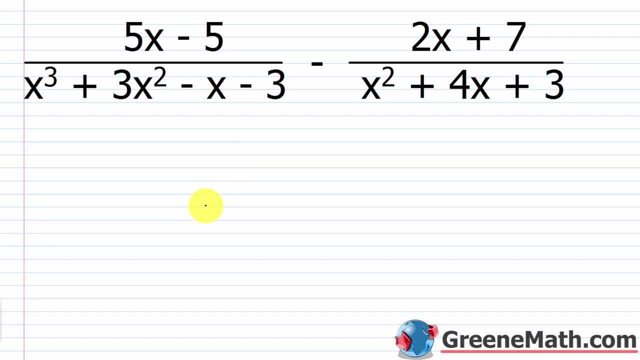 the end. I want you to have some practice doing that. So I have 5x minus 5 over x cubed, plus 3x squared minus x minus 3, minus 2x plus 7 over x squared plus 4x plus 3.. So if you see minus, 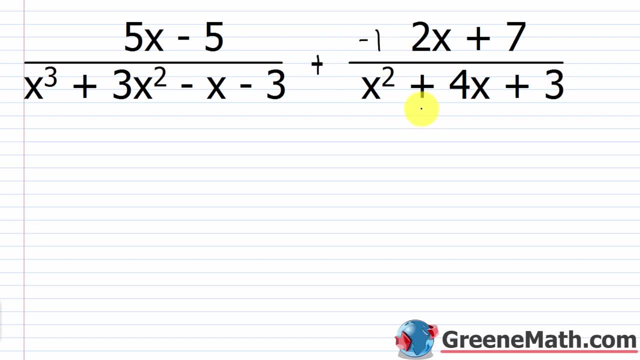 just put plus and then negative 1.. So this negative 1 is going to multiply by the numerator. Remember, if it's a fraction, I don't put negative 1 in the numerator and the denominator because those would cancel. So you just want a negative 1 either in the numerator or the denominator. 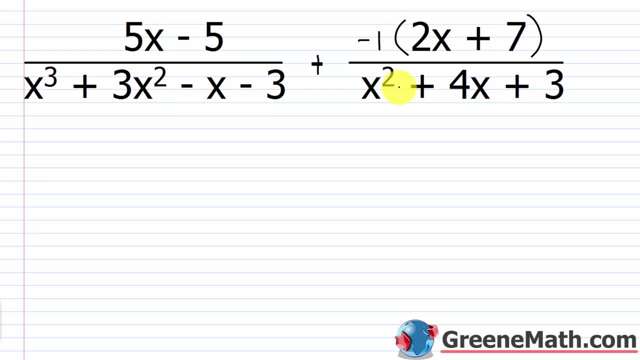 Preferably you're going to do it in the numerator. You don't want to mess up your denominator because you need to get a common denominator. You don't want to mess with that. So just put plus and then negative 1 times your numerator, and then you can forget about the messy subtraction. 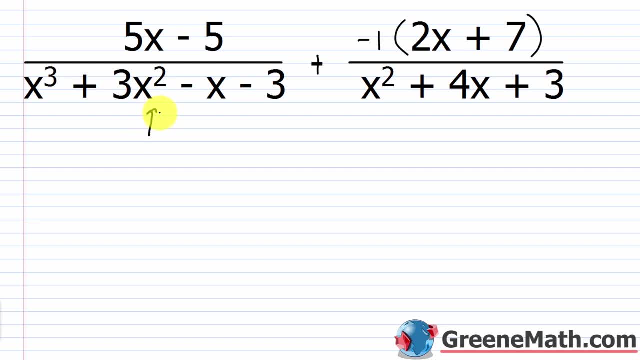 All right. So for my denominator in this one I can use factoring by grouping. I have a four-term polynomial From the first group. I could pull out an x squared, and that would leave me with x cubed. So I'm going to put x cubed over x cubed, And that would leave me with x cubed over. 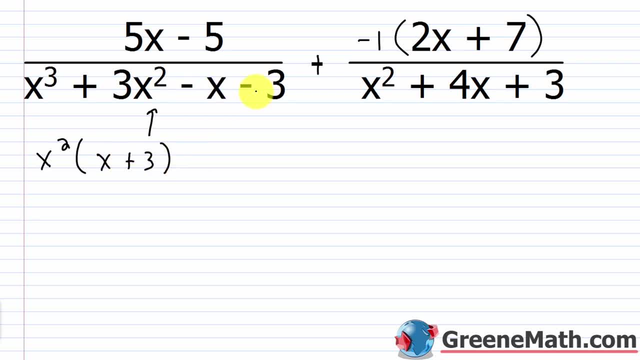 x cubed. So I'm going to put x cubed over x cubed And that would leave me with x cubed over x cubed, And that would x plus three. In the second group I could pull out a negative one and that would leave me with. 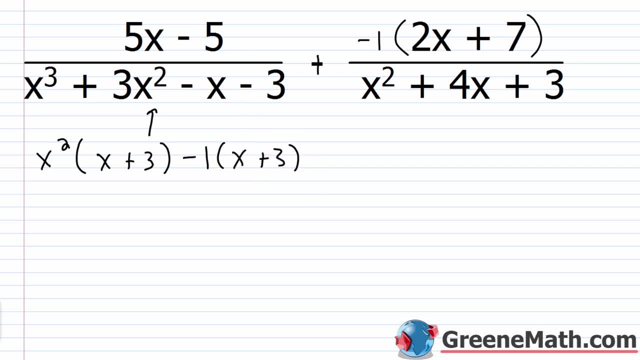 x plus three. If I factored out the common binomial factor of x plus three, this guy would factor into what You'd have the quantity x plus three times the quantity x squared minus one. Now, x squared minus one. you might not notice this, but that's what. That's the difference of. 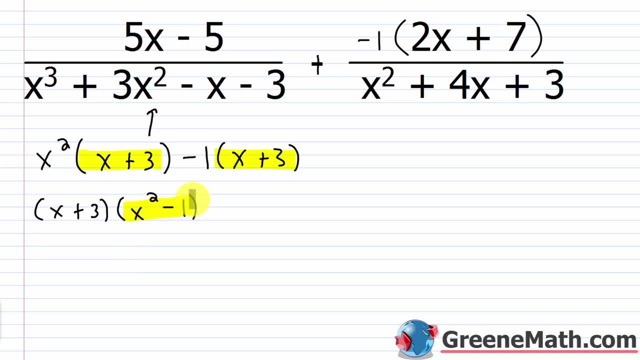 two squares, So this can be further factored. So really this is x plus three times the quantity x plus one times the quantity x minus one. Always look for further factoring. This is something I see on tests all the time, where you get x squared minus one, just left like this: 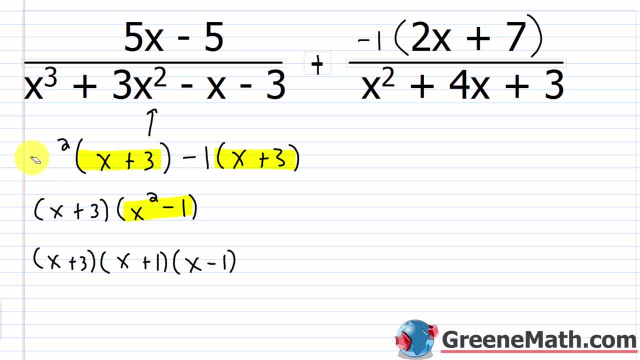 and the student just kind of moves on. So let's just erase all of this and we'll bring this up here. This is x squared minus one, and this is x squared minus one is our factor denominator. Now, to factor this denominator, I'm going to set this up as the 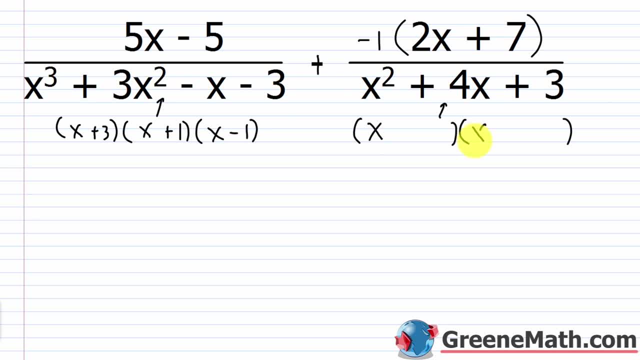 product of two binomials. I'll put x here and x here, And then I want two integers whose sum is four and whose product is three. So we know that would be plus three and plus one. Now I have over here x plus three and x plus one, So those are common to each. So really, all I'm missing is this: 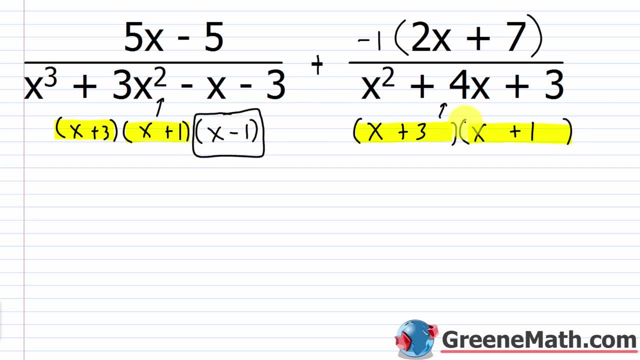 x minus one here over here. So this guy right here can stay as it is. I can keep five x minus five as it is, And all I really need to do is take this guy right here and multiply the numerator and denominator by what I'm missing, which is x minus one. So let's put equals. We've got this. 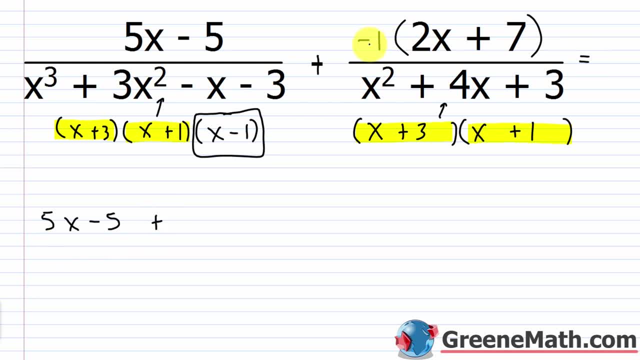 I'm going to put plus First. I'm going to use my distributive property. Negative one times two x is negative two x. And then negative one times seven Is minus seven. So it would be this, multiplied by this, What I'm missing, this quantity x minus one. 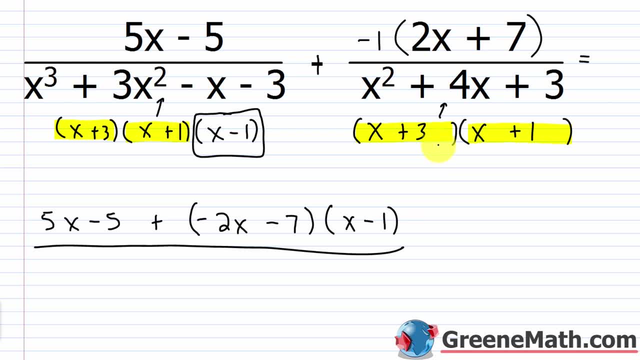 Okay, so now that I have that set up, this is over my common denominator, which is x plus three, that quantity times x plus one, that quantity times x minus one. So again, all I did was I multiplied the numerator here by x minus one, which I'm doing right there. That's the multiplication. 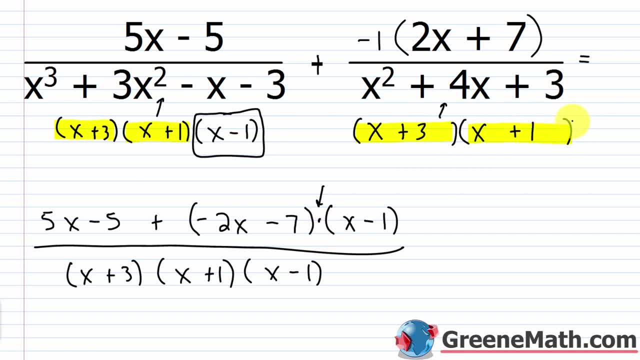 And I multiplied the denominator, although I didn't show you that I'm multiplying the denominator by x minus one. also, If I did that down here, I would have that common denominator that consists of x plus three, that quantity times x plus one, that quantity times the quantity x minus one. So that's where I got that. 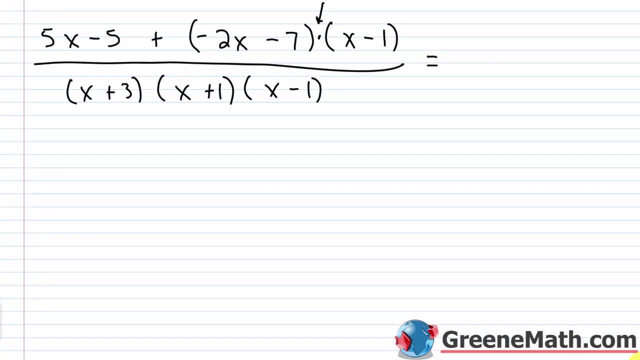 All right. so now that we fully understand, let's kind of scroll down, Let's complete this process. So we've got five x minus five And then plus. we want to use FOIL here. So negative two x times seven is negative two x minus five. So negative two x times seven is. 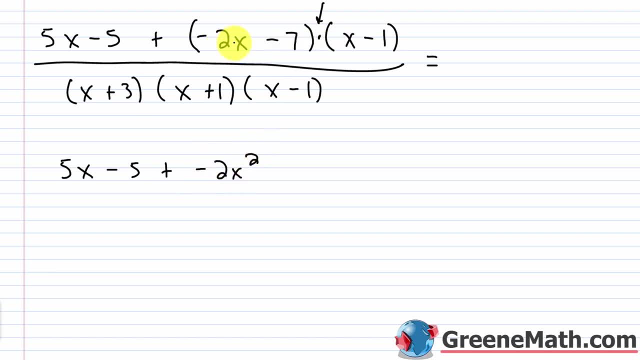 negative two x squared, Then negative two x times negative. one is positive two x, Then negative seven times x is minus seven. x, Then negative, seven times negative. one is plus seven. So let me write this over that common denominator: We've got the quantity x plus three times the. 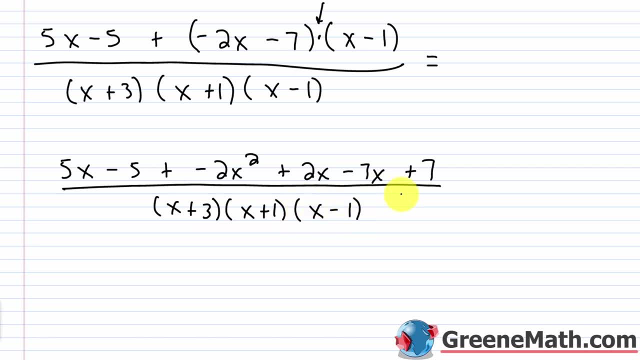 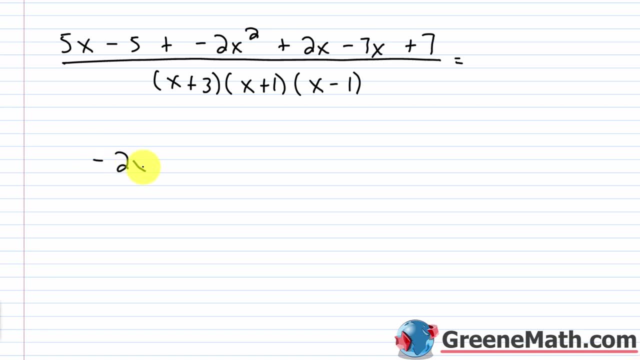 quantity x plus one times the quantity x minus one. All right, In the numerator I've got my leading term of negative two x squared. Nothing to combine with that. I've got five x, two x and negative seven x. Five x plus two x is seven. 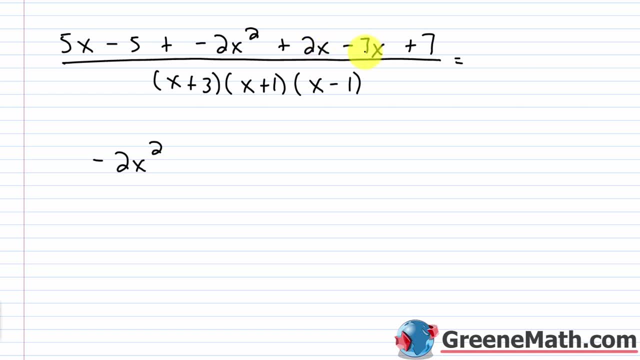 x Seven, x minus seven, x is zero. Then I'm just left with negative five plus seven, which is positive two. So this is over. We've got the quantity x plus three times the quantity x plus one times the quantity x minus one, And I promised you that we could finally cancel something. 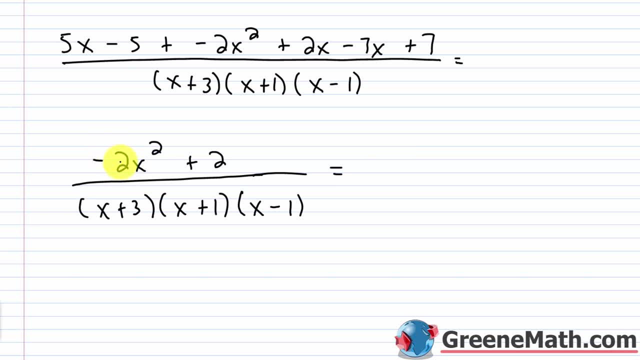 So in the numerator, if you look, if I were to pull out eight x plus one times the quantity x minus one, I would have to do the same thing If I had a negative two. what would that leave me? I would have negative two times, in parentheses. 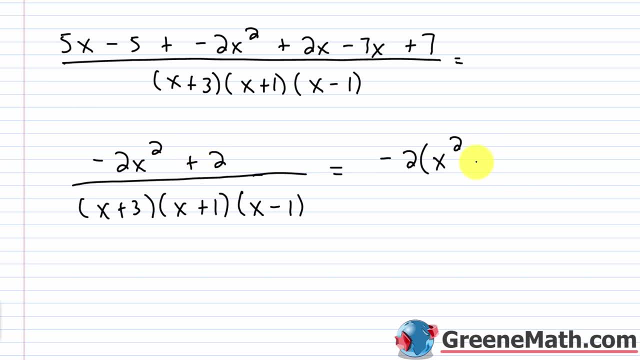 I'd be left with x squared. The sign here would change, So it would be minus, And if I pulled out a two it would be one. Now remember: x squared minus one, that's the difference of two squares. So I can further factor that into the quantity x plus one times the quantity x minus. 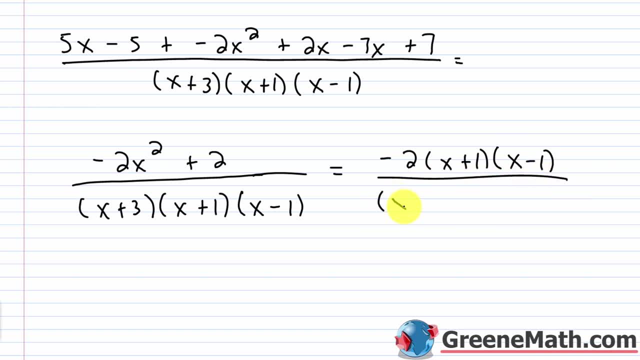 one And this is over. So we'll have the quantity x plus three times the quantity x plus one times the quantity x minus one. So look at what we can cancel. We can cancel this x plus one with this x plus one, and this x minus one with this x minus one, And in the end I'm left with a negative. 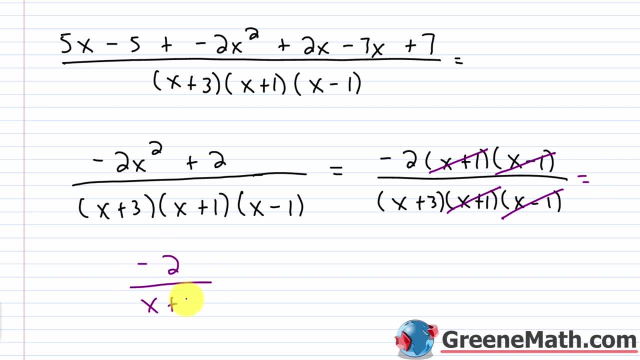 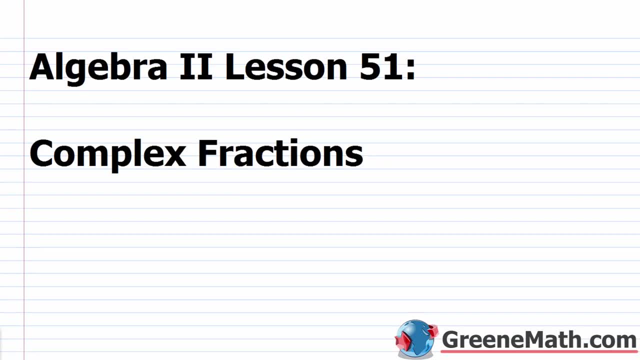 two over the quantity x plus three. You don't need to put parentheses around it, You can just leave it as it is. So this is going to be my simplified answer. Hello and welcome to Algebra 2, Lesson 51.. In this video, we're going to learn about complex fractions. So again, we talked about 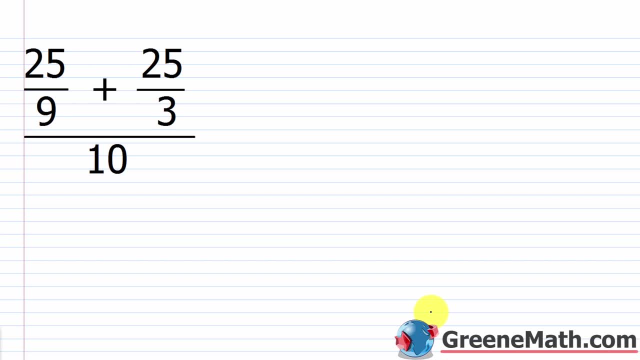 this back in Algebra 1.. We're going to learn about complex fractions. So again, we talked about this back in Algebra 1.. We're going to learn about complex fractions. So again, we talked about this back in Algebra 1.. And for the majority of stuff with regard to rational expressions, we've already 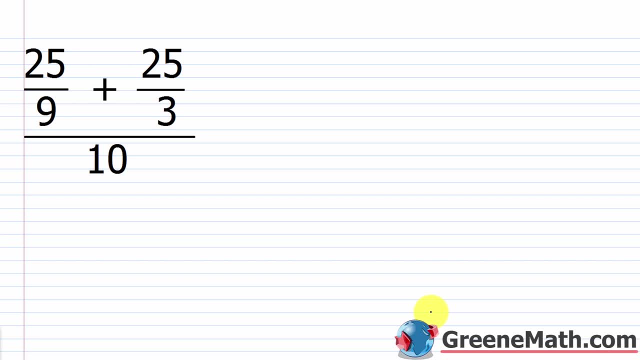 seen it before. So how would we simplify something like this? Well, first and foremost, we know it as a complex fraction, That's a fraction where there's another fraction in either the numerator, the denominator, or both the numerator and the denominator. Well, we really have two methods to. 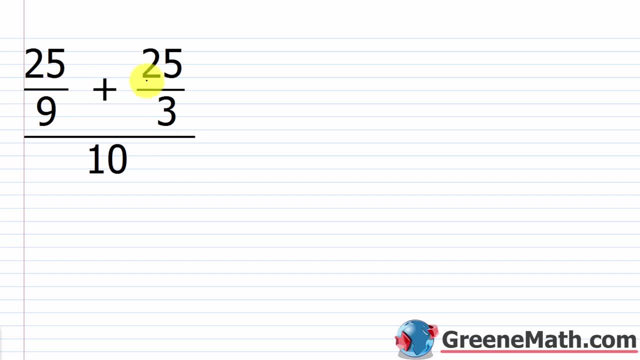 kind of work with this. The first method would be to attack kind of the numerator and denominator separately, Then to do kind of the main division. So this would be your main division or your main fraction bar. Let me kind of make that arrow a little better. So what I could do here is I could say, okay, well. 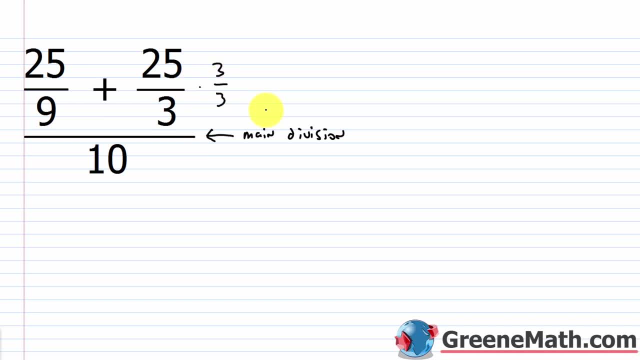 I need a common denominator. So I could multiply this by 3 over 3. And so this would give me what I would have: 25 plus 75 over 9. And then this is over 10.. 25 plus 75 is 100.. So you would basically. 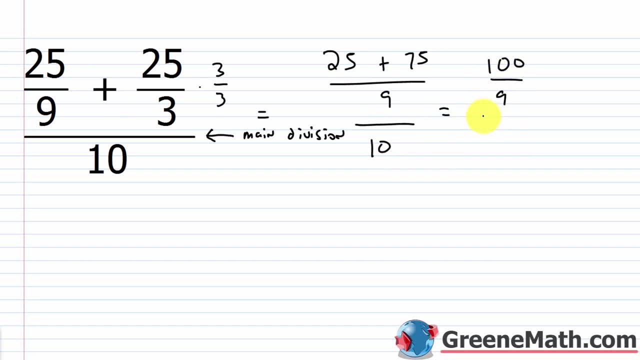 have 100 over 9.. You think about this as divided by 10. And you could do 10 over 1 if it makes you more comfortable with the process. Because what do we do? We take the first fraction, which is 100. 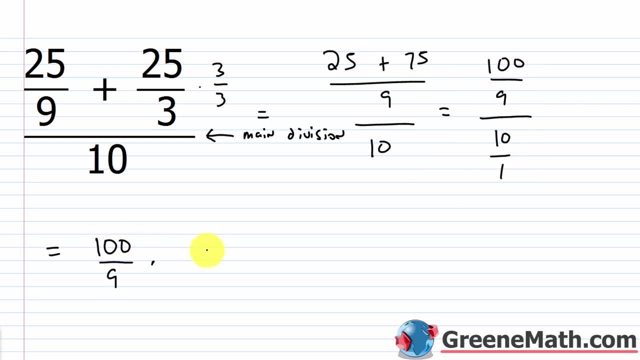 over 9.. And we multiply by the reciprocal of the second fraction, which is 1 over 10.. So I can see that I can cancel this with this and I get a 10.. And so I end up with what? 10 ninths? 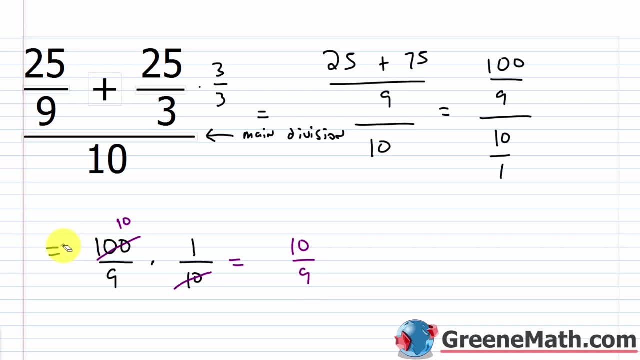 So what's the other way to kind of do this Kind of the faster way, At least in most scenarios? Well, you can find the LCD for all the denominators involved. Okay, so, for all the denominators involved. So I have a 9,, I have a 3, and I have a 10.. 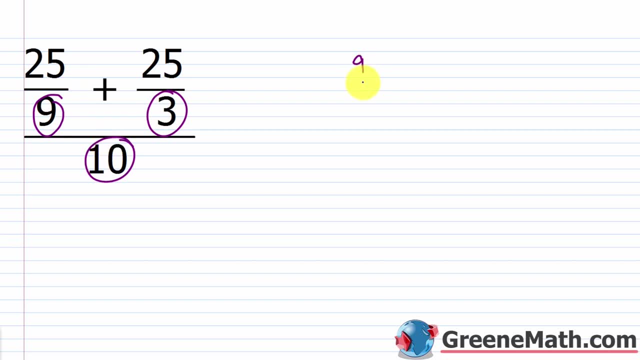 So what's the LCD? Well, 9 is what It's 3 times 3.. 3 is prime and 10 is 2 times 5.. Okay, so what I would do is I would include each different factor. 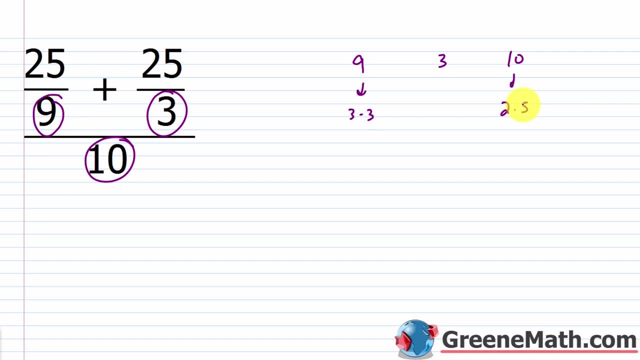 up to the largest number of repeats. it appears in any factorization. So here I have 3 times 3,, here I have 3.. So it appears twice in the factorization of 9,, only once here. So my LCD would include two factors of 3 or 9.. Then times I have 2, doesn't appear anywhere else, so it just. 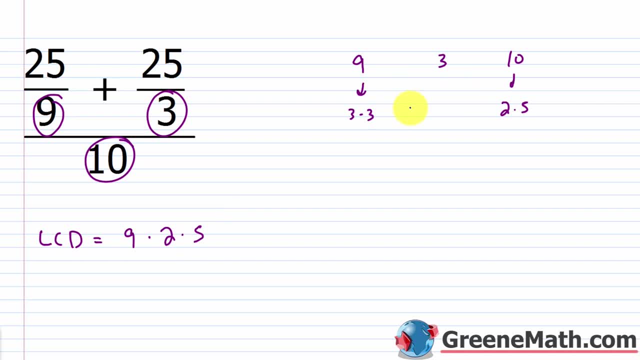 goes in there, Then times 5, again doesn't appear anywhere else, so it just goes in there. 9 times 18,, 18 times 5 is going to give us 90. So what I would do is I would multiply the numerator and denominator of the complex fraction by 90.. Now this is where 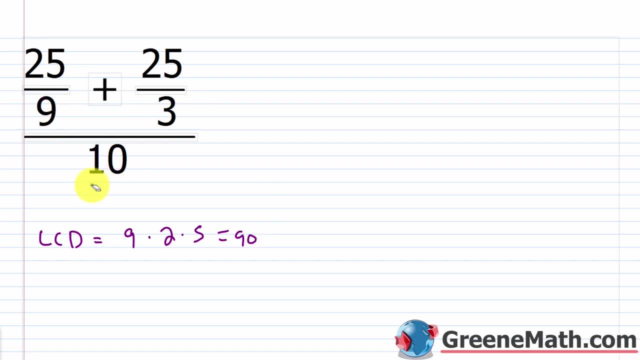 it gets a little complicated because you're like: well, what's the numerator and denominator of the complex fraction? Again, if this is the main division, I could multiply this by 90 and this by 90. And so what's going to happen? Let me just erase this real quick. Again, I'm just multiplying. 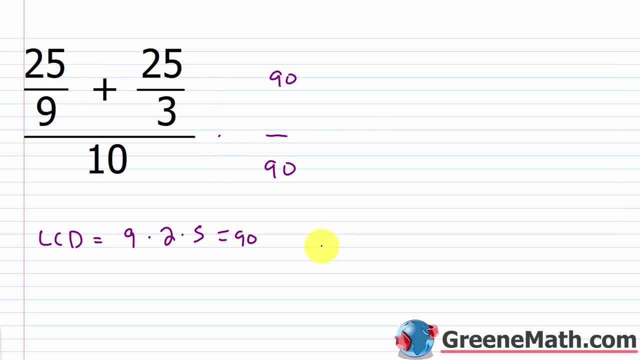 by 1, and let me make these into 1 multiplication symbol, And 90 over 90 is 1.. I'm allowed to do that. So what would this give me? Well, if I distributed this 90 to this 25 over 9, the 90 would cancel with the 9 and give me a. 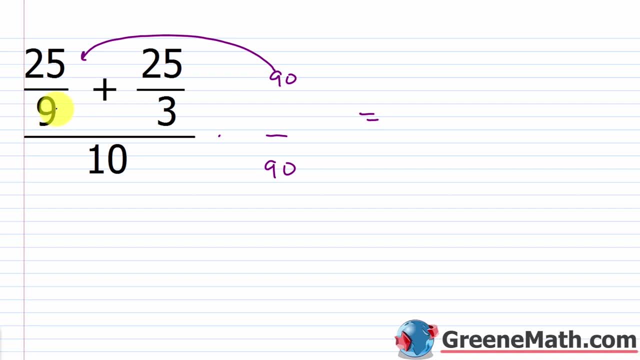 10.. So I would basically have 10 times 25, which is 250.. Then, plus, I'd do the same thing again: 90 times 25 over 3.. 90 would cancel with 3 and give me 30.. 30 times 25 would give me. 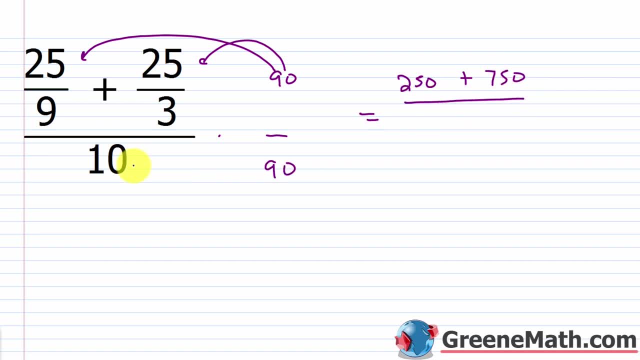 150.. Then this would be over 90 times 10, which would be 900.. So what does this leave me with? It looks like it's not going to work out, but it will. 250 plus 750 is 1,000.. This is over 900. 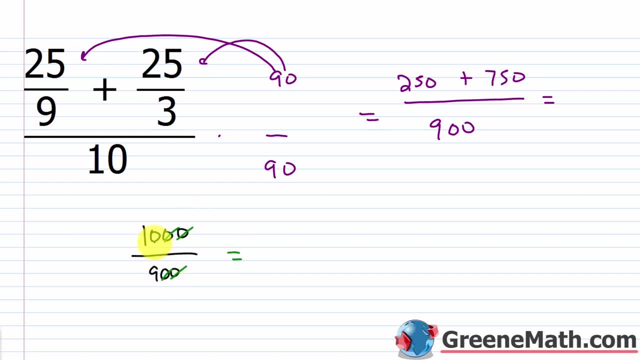 Well, if I just cancel two zeros, I end up with what? 10 ninths, just like I saw with the other method. So really, it doesn't matter what you use, It's just a matter of what you're more comfortable with Now. this is a very easy way to do this. You can do this with any of your 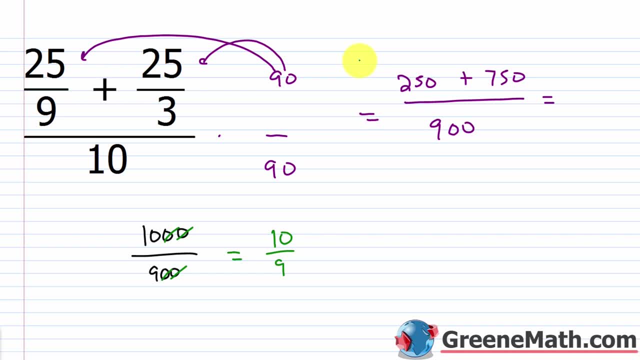 equations. So this is a very easy scenario to deal with because we're working with just regular fractions. When we turn up the heat here and we look at these complex fractions that have rational expressions in them, it's going to be a little bit more tedious. So let's look at 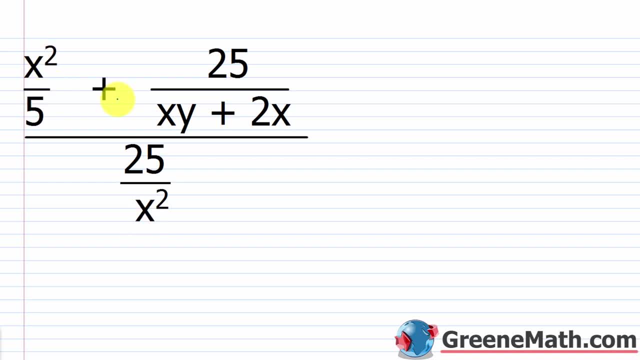 the first scenario here where we have x squared over 5 plus 25 over xy, plus 2x over 25 over x squared. So this is your main division. This is your main division. I can go through and I can get common denominators here. I can do the addition. 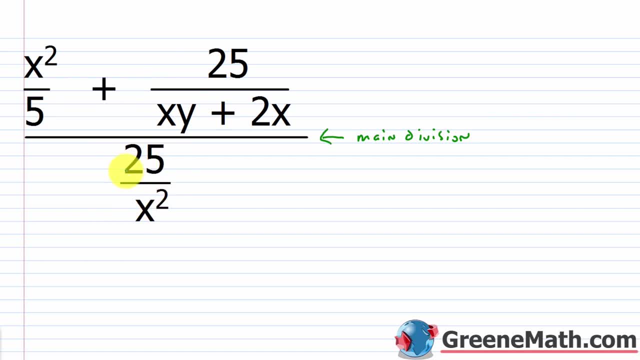 and then I can do the division with this. But I'm going to tell you right away: the LCD method is generally- this isn't every time- but it's generally going to be faster when you're doing these with rational expressions. It just is. So let's just focus on that. 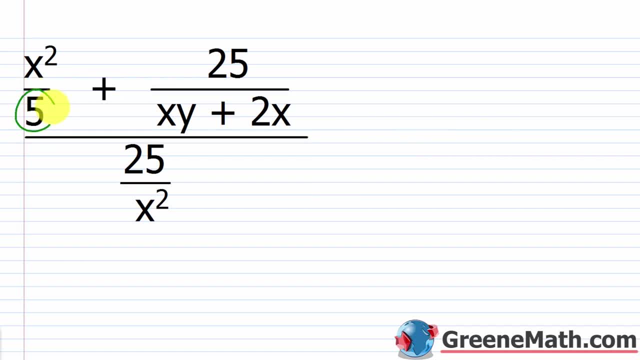 What is the LCD for all denominators? I've got a 5. So throw that in there. I've got an xy plus 2x. This could be factored into what x times the quantity y plus 2.. So we'll multiply this by. 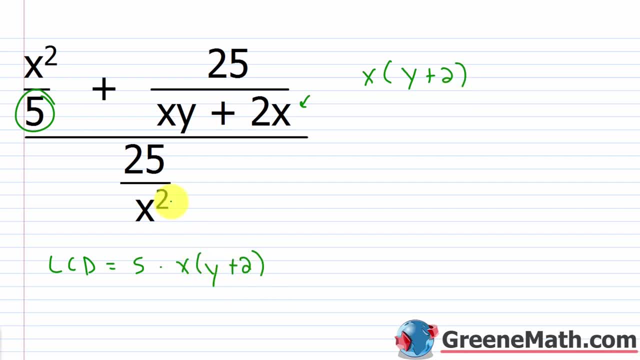 x times the quantity y plus 2.. And then this one is just x squared. I've already got an x here. Do I need x cubed? No, I do not, Because if I broke this down, this would be x times x. 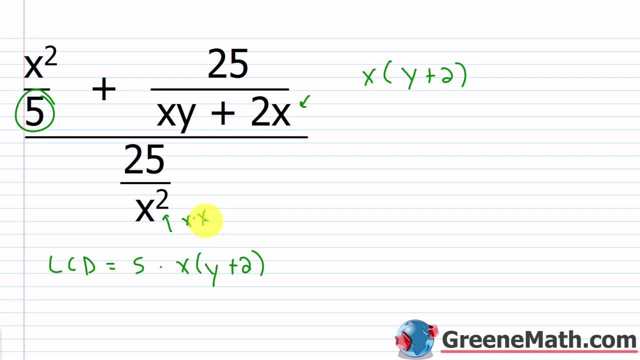 and this would be x, So I'll go with the largest number of repeats. So all I'm going to do is make this x squared. Okay, Please don't make the mistake of saying, okay, I've got one x here and I've got an x and another x, So this is x cubed. It doesn't work that way Again. 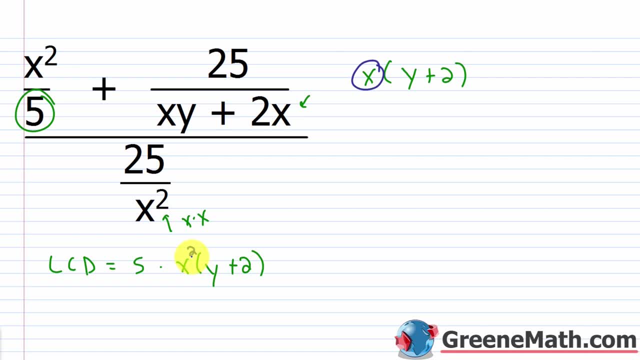 the largest number of repeats. in this case that's going to be two of them. So my LCD is what? It's just 5x squared. I'll put these together: 5x squared times the quantity y plus 2.. So if I just multiply the numerator, which is this guy right here- I'll put it in parentheses- 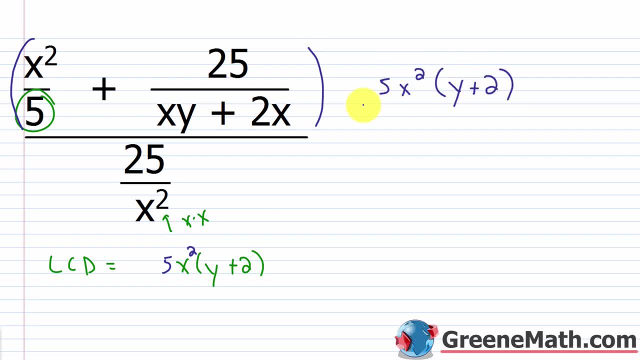 5x squared times the quantity y plus 2.. If I multiply my numerator by this and my denominator by this, this is my denominator. I'll be able to just simplify this. All right, So I'm going to put my multiplication symbol and now we're ready to go. 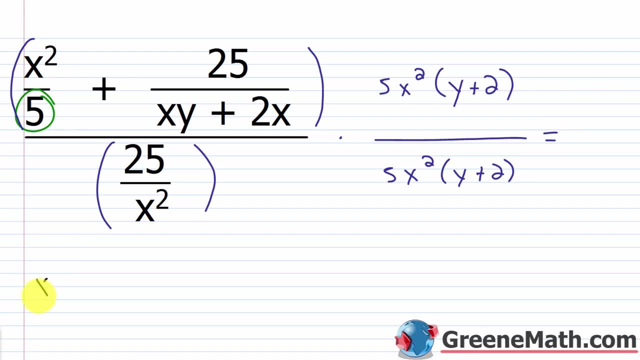 So I will have what I will have: x squared over 5, multiplied by 5x squared times y plus 2, right That quantity. You can see that these 5s would cancel, and so what I'm left with is x squared times x squared, which would be x to the fourth power. 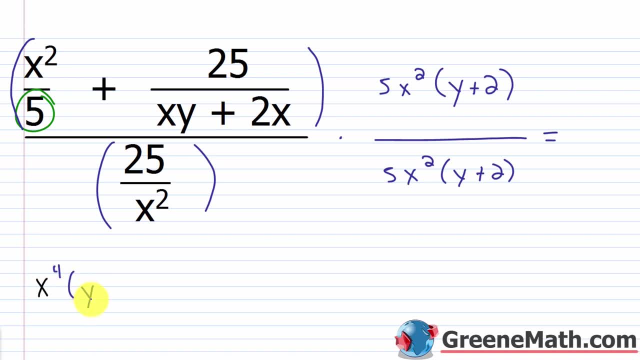 Let's go ahead and write this as x to the fourth power times the quantity y plus 2.. Now then I have plus. I'm going to multiply this times this, So we'd have 25 over in factor form. that's x times the quantity y plus 2. times we have 5x squared times the quantity y plus 2.. 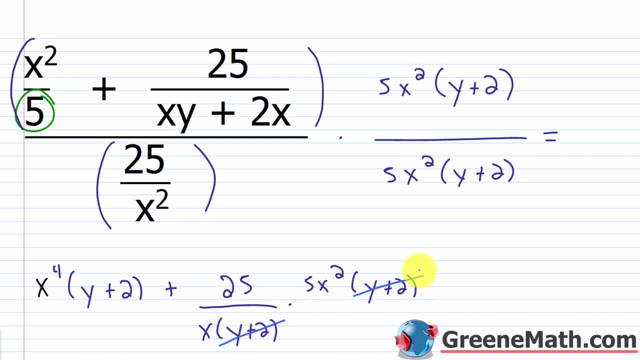 So what's going to happen is this is going to cancel with this. This will cancel. with one of these, I'll have 25 times 5, which is 125 times x. So plus 125x. Okay, then, this is over. Now for this one. if I multiply this by this, 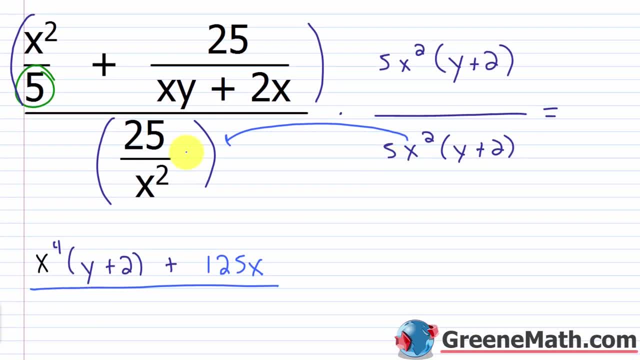 we know, just the x squared would cancel. So I'd be left with 5 times 25,, which is 125, times the quantity y plus 2.. Now, anything I could factor out from the numerator. Well, I could pull out an x, right, if I wanted to. 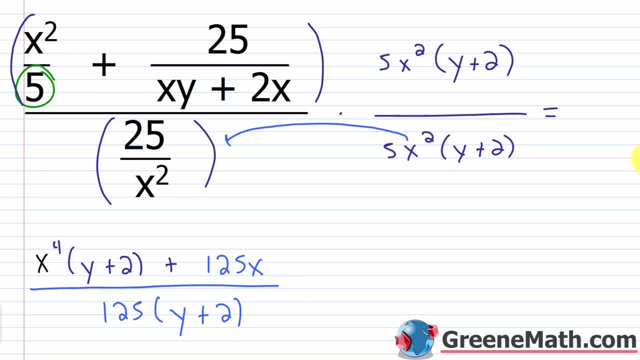 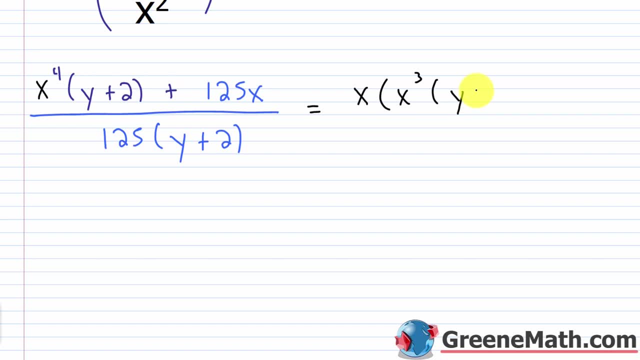 So let's just go ahead and do that. You want to try to leave these things in factored form if you can. So if I pulled out an x, I would have x cubed times the quantity y plus 2, and then plus 125. 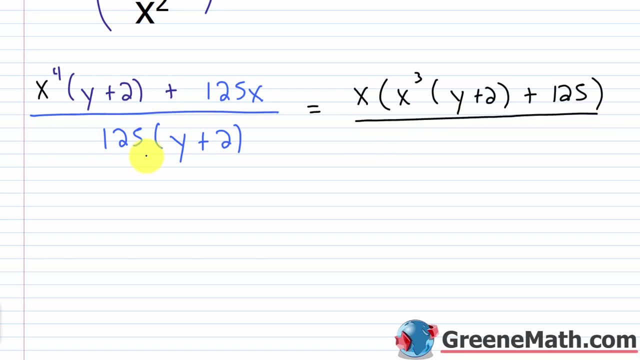 And then this is over. So we'd have 125 times the quantity y plus 2.. Nothing else I can really do to to factor, Nothing I can really cancel. I just leave it like this so that it's obvious I can't. 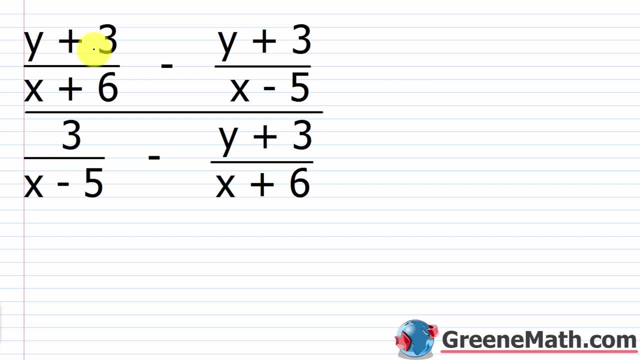 cancel anything else. Well, let's take a look at another one. So we have y plus 3 over x plus 6 minus y plus 3 over x minus 5.. Then this is over. We have 3 over x minus 5 minus y plus 3 over x. 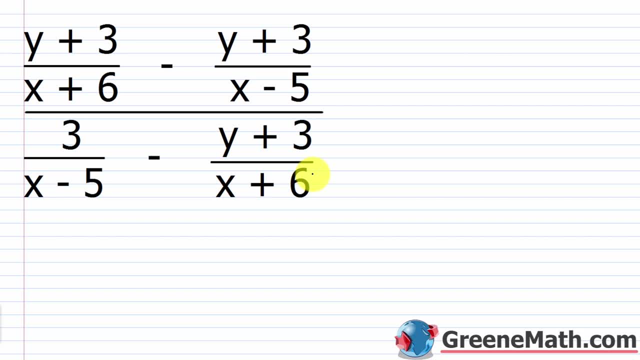 plus 6.. So for the LCD it's going to be 1.. The LCD is 1.. Nothing can really be factored. We would just list things. So I have an x plus 6 here and here. So only one of these things is going to be. 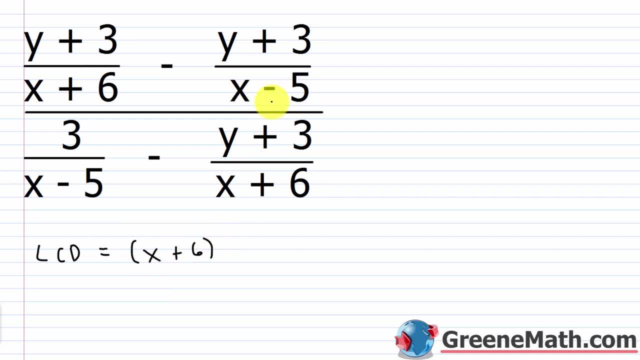 in when I build my LCD, Then I have an x minus 5 here and here, So again, only one of those goes in when I build my LCD. So what I'd want to do is multiply the numerator of the complex fraction, which is going to be this up here, and the denominator of the complex fraction, which is: 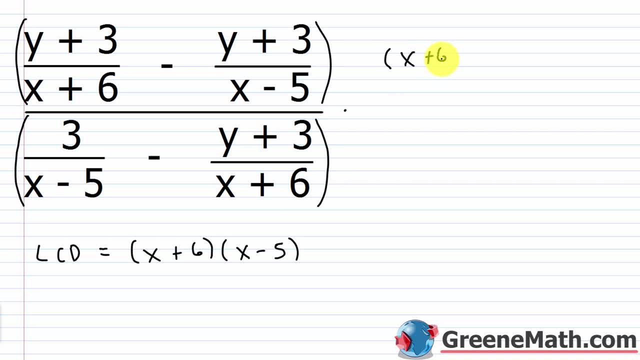 this down here by this quantity x plus 6 times the quantity x minus 5.. So this is x plus 6 times x minus 5.. All right, So if I use my distributive property here, I can distribute this to this, And so what? 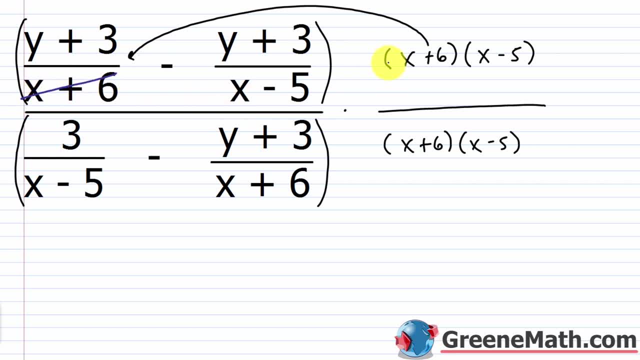 would happen here. We need to write everything out. This is going to cancel with this. So what I'm going to have is x minus 5, that quantity times the quantity y plus 3.. Let me erase this and this. If I did the same thing here now- x minus 5, that would cancel with this. I'd have. 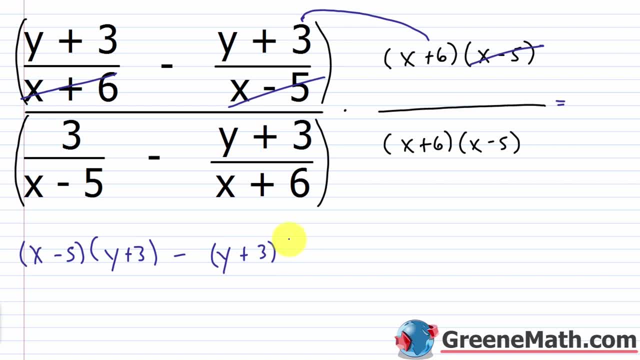 minus, you'd have y plus 3, that quantity times the quantity x plus 6.. Now that minus is important. I'm subtracting all of this away. You can put this in brackets if you want to make it crystal clear Or if you're good enough to remember that you can leave. 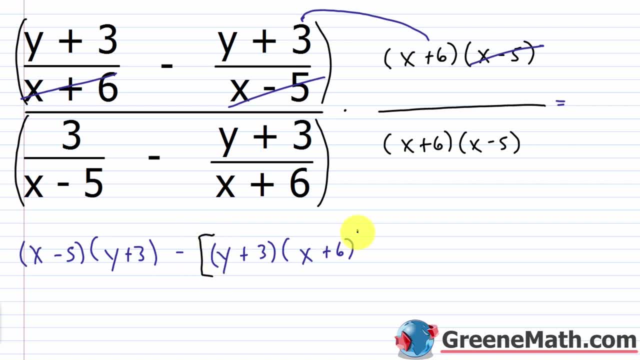 it alone. But I think it'd be important here to just put it in brackets, That way we don't make a simple sign mistake. All right, Then this is going to be over 1.. So I'm doing the same process here. So this would get multiplied by 1.. So I'm going to have x minus 5, that. 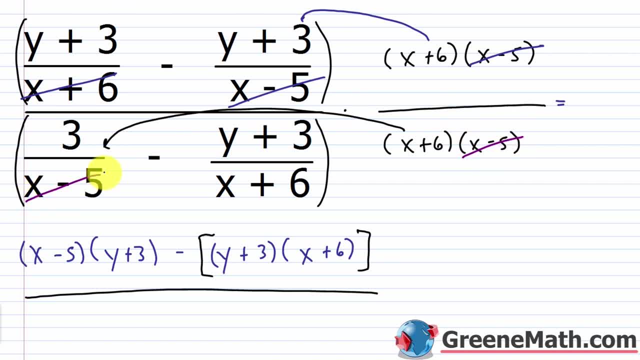 would cancel with this The x minus 5, that would cancel here and here. So you would have 3 times the quantity x plus 6.. Then minus. If I erase this and this, this would get multiplied by this. So this would cancel with this And I would have y plus 3, that quantity multiplied. 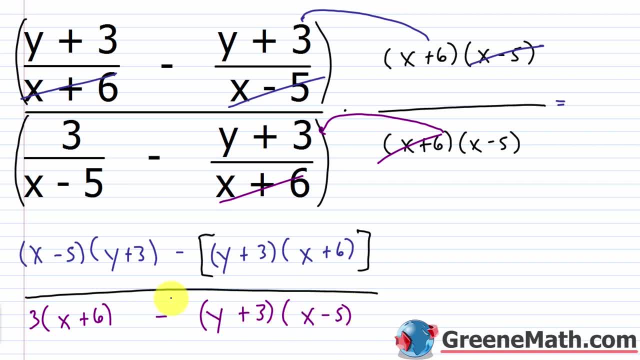 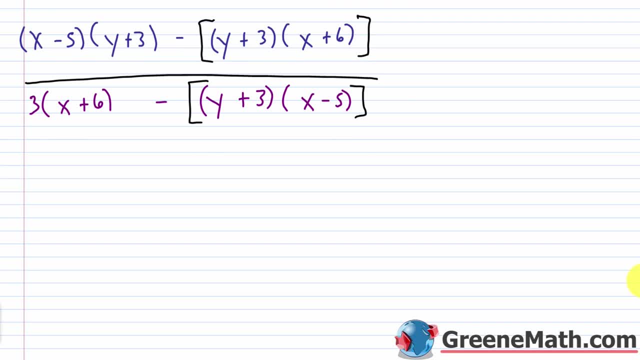 by x minus 5, that quantity, Again we have that minus sign. So let's put it inside of brackets. Okay, So let's scroll down a little bit. Now. what should we do here? Let's go through and do our multiplication and see what we can cancel, what we can get rid of x times. 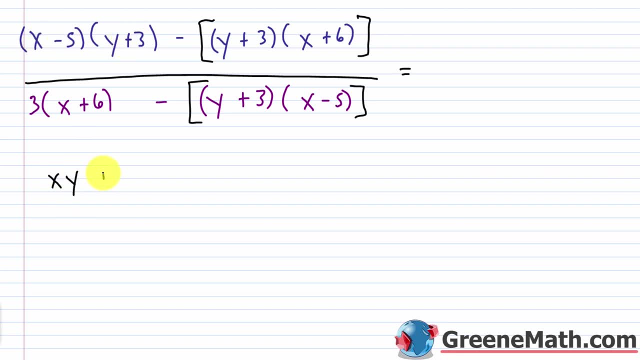 y is xy. x times 3 is plus 3x. Negative 5 times y is minus 5y, And then negative 5 times 3 is minus 15.. Now I'm going to put minus and I'm going to put my brackets there and 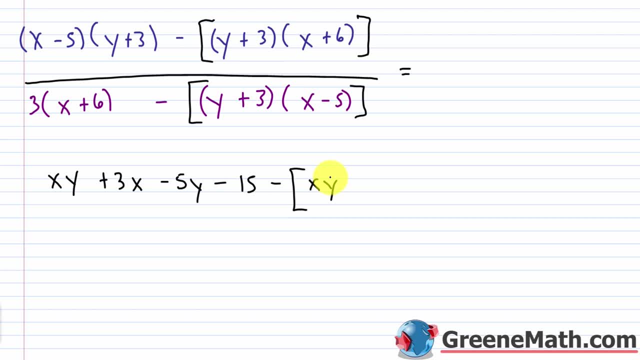 I'm going to do my multiplication: y times x is xy, y times 6 is plus 5y, And then negative 5 is plus 6y, 3 times x is plus 3x, And then 3 times 6 is plus 18.. So then, this is over. 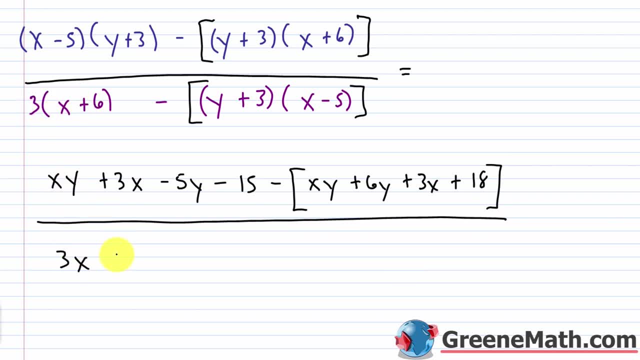 We have 3 times x, which is 3x, Then 3 times 6,, which is plus 18. And then, right here we put minus And then inside of brackets, y times x is xy, And then y times negative 5. 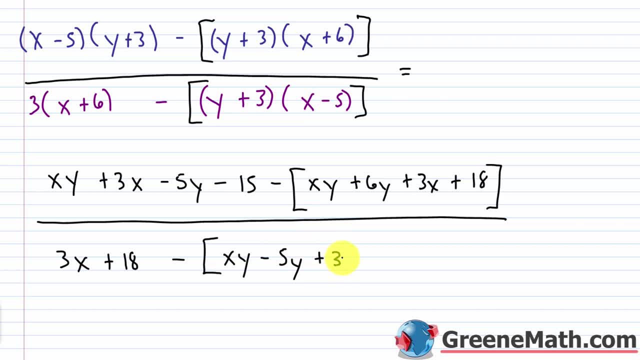 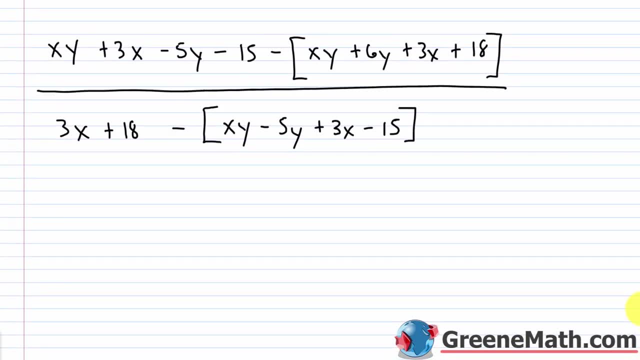 is minus 5y, And then 3 times x is plus 3x, And then 3 times negative 5 is minus 15.. So we're going to do our multiplication. Okay, All right, Let's scroll down and get a little room going. So what can I do here? So let 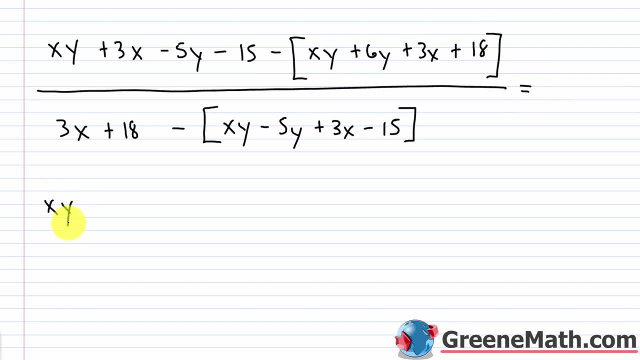 me just start out by just doing this: I have xy, I have plus 3x, I have minus 5y, I have minus 15.. Now this minus is going to get distributed to every term inside the parentheses. We don't want to make a sign mistake. So this would be minus xy, It would be minus. 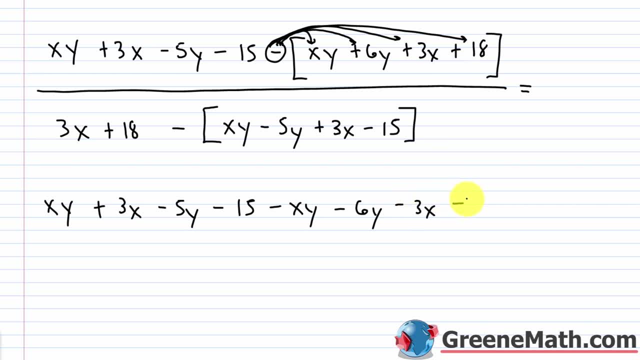 6y, It would be minus 3x, It would be minus 18.. Okay, And we'll come back and simplify that in a second and make that a little bit better. Down here I have 3x plus 18.. And then I'm doing the same thing: I'm going to distribute. 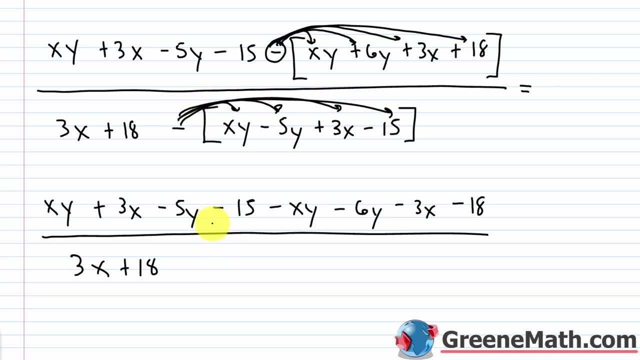 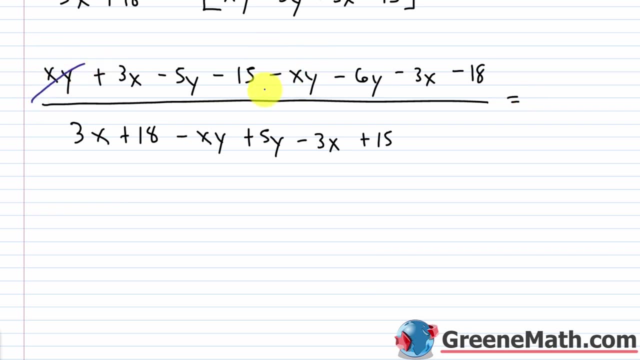 this to every term, every term. So I'll have minus xy, I'll have plus 5y, I'll have minus 3x And I'll have plus 15.. Okay, So we have xy minus xy. Those would cancel. Just d ride these two over. Should just do. 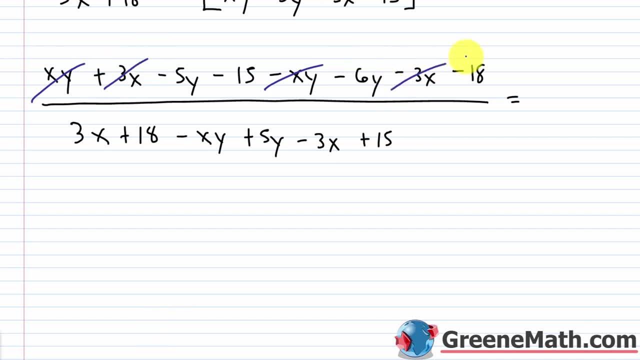 get rid of that. you have 3x and you have negative 3x, those cancel. get rid of that. you have minus 5y. minus 6y, those would give you minus 11y. i have negative 15 and minus 18, so that's going to give. 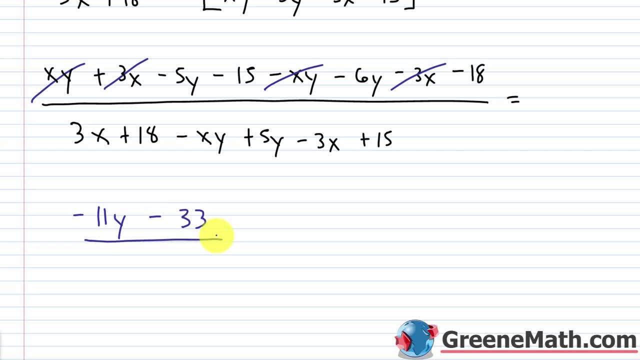 us negative 33. so then this is over down here. what can we cancel? again, we have 3x and negative 3x. that cancels. so we'd have negative xy plus 5y and then 18 and 15 would be 33. so can we do anything to factor the numerator? well, i could pull out an 11 or a negative 11. 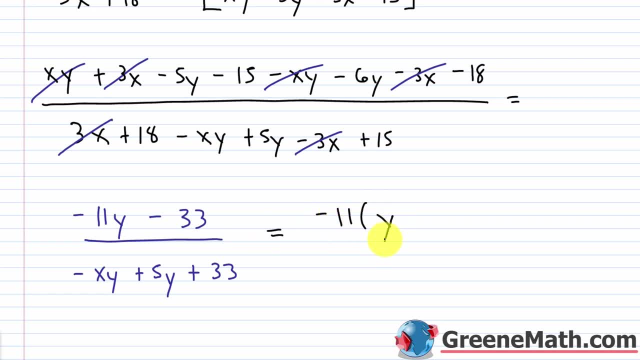 let's just pull out a negative 11. that would give me y plus 3 in the denominator. could i pull anything out? could i factor anything? the answer to that is no, so i'm just stuck with this negative 11 that cancels. so we'd have negative xy plus 5y, and then 18 and 15 would be 33. 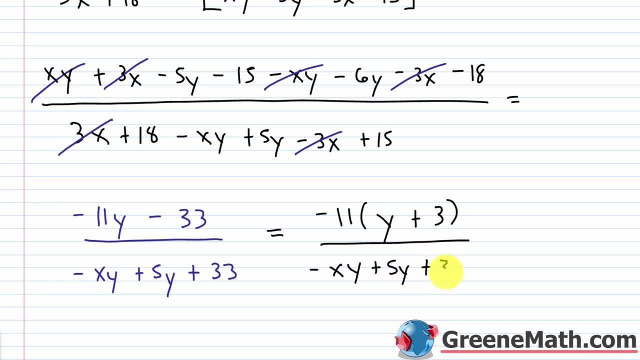 negative xy plus 5y plus 33, and this is the best that we can do. right, we could do different variations of that. we could leave it like this: i could have pulled out a positive 11 from the numerator. you know all kinds of things that we could have done, but really that's the answer. so 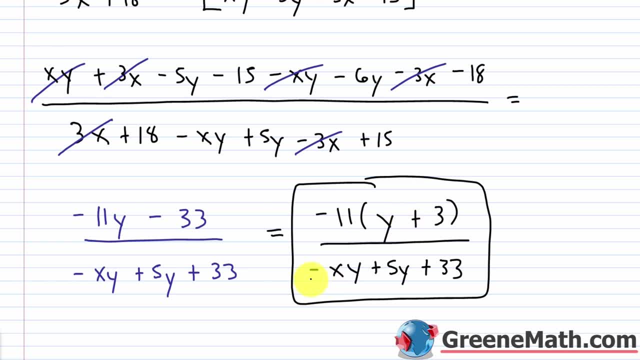 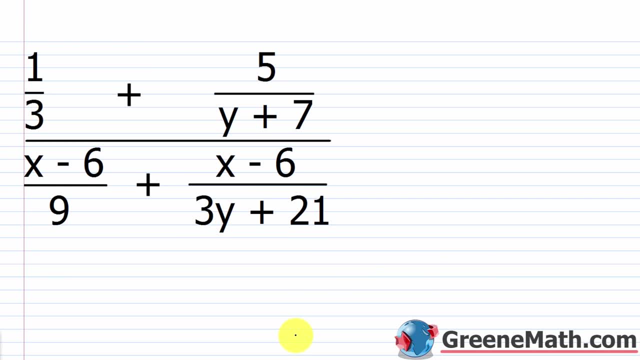 we have negative 11 times the quantity y plus 3 over negative xy plus 5y plus 33. all right, let's take a look at one more of these again. i think this is something that most of you already know how to do. we have one third plus 5 over y plus 7, and this is over. we have x minus 6 over 9 plus x. 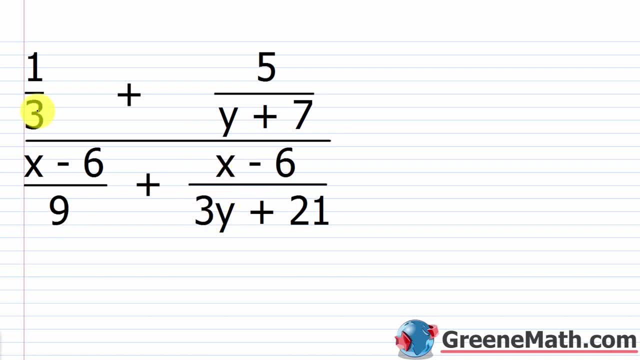 minus 6 over 3y plus 21. so 3, i can't factor y plus 7. i can't really factor 9. i could factor into 3 times 3 and then 3y plus 21. i could factor into 3 times the quantity y plus 7. so what do i have? 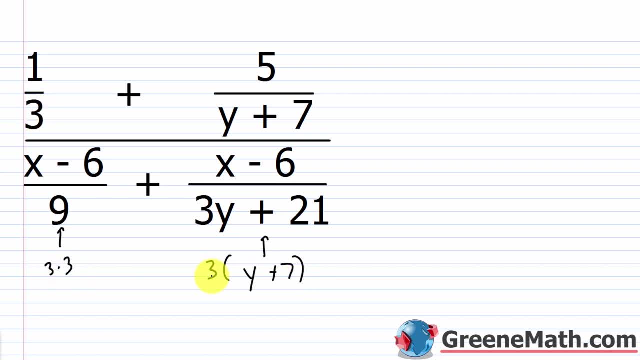 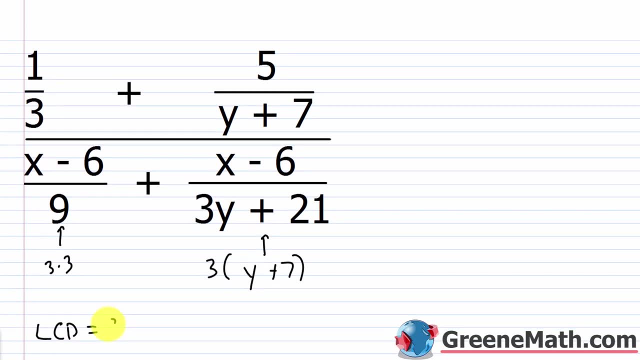 here. i have a 3 here, two threes here and a 3 here. so if i'm building a building, a Building, my LCD, I would put two 3's in, because that's the largest number of repeats, so I'd put 9 there. 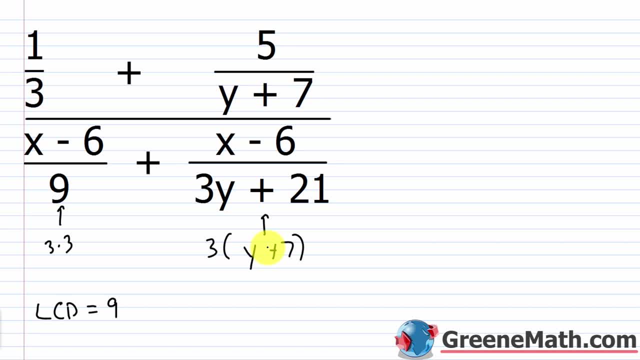 Then I have a y plus 7 and a y plus 7.. It only occurs once in each of those, so I just gotta put one in. So once I have my LCD, it's very, very simple. Just again: multiply the numerator of the complex fraction by 9 times the quantity y. 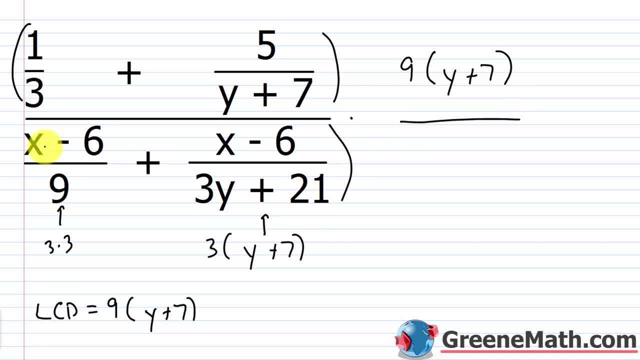 plus 7, and do the same thing to the denominator. so we're multiplying by 9 times the quantity y plus 7.. Alright, so let's erase this and we can get started. So multiply this by this. We know that 9 would cancel with 3 and give me 3.. 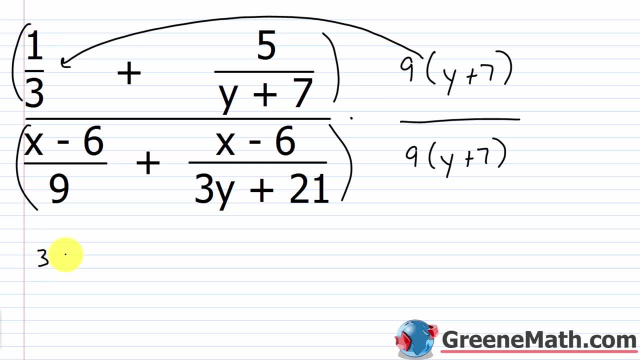 The only thing we have up here is a 1, so it would basically be 3 times the quantity, y plus 7, then plus, if I use my distributive property here, the y plus 7's would cancel. So this would cancel with this and I'd be left with 9 times 5, which is 45.. 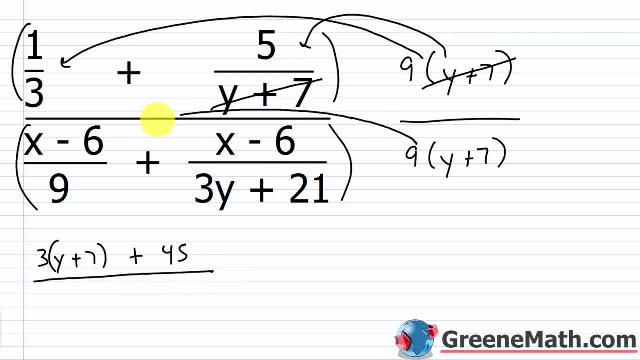 Okay, In the denominator we use our distributive property, the 9's would cancel. you'd have x minus 6, that quantity multiplied by the quantity y plus 7, then plus The next thing we'd see: we would multiply this by this. now again, this factors into: 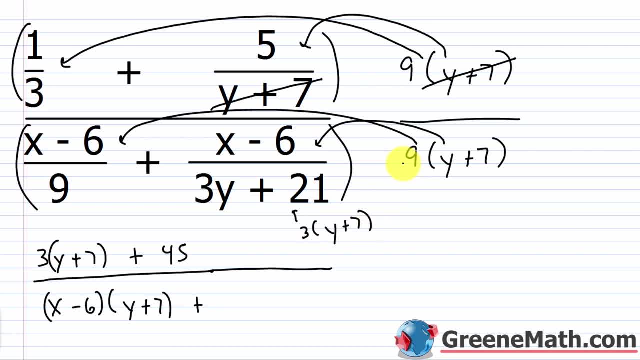 3 times the quantity y plus 7.. So what would happen is the 9 would cancel with a 3 and give me a 3, and the y plus 7's would cancel. You would essentially have 3 times the quantity x minus 7.. 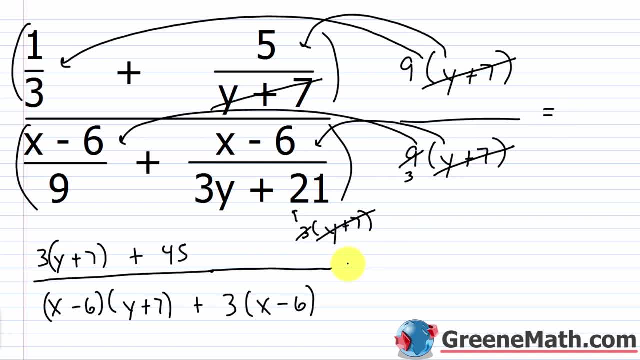 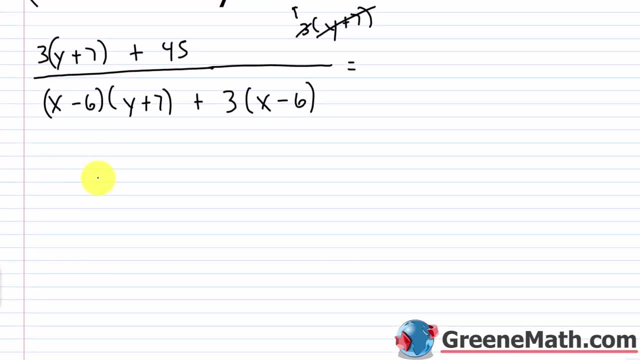 Let me put my equals here. and put equals here, and then let's scroll down a little bit. So in the numerator 3 times y is 3y, plus 3 times 7 is 21, and then plus 45.. 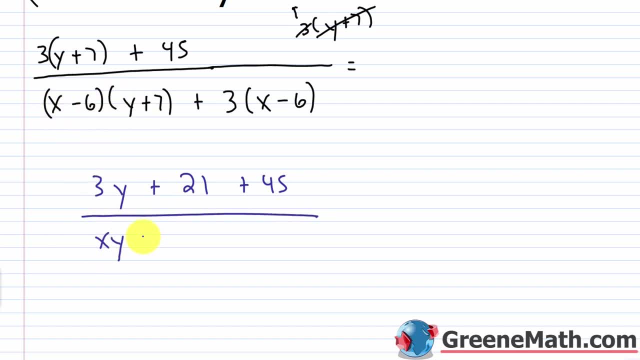 In the denominator x times y is xy, then x times 7 is plus 7x, then negative 6 times y is minus 6y, then negative 6 times 7 is minus 42. Then plus 3 times x is 3x, and then 3 times negative 6 is minus 18.. 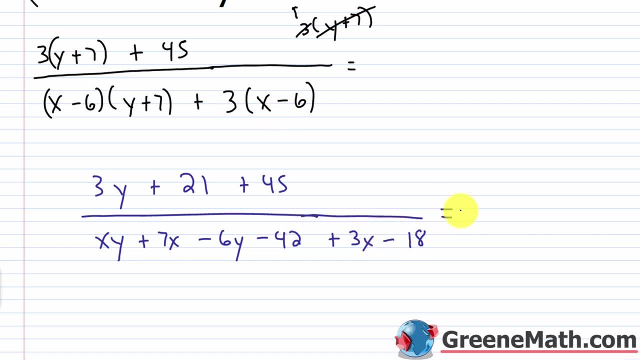 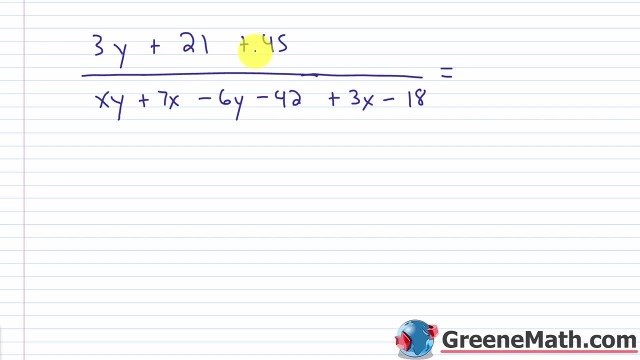 All right, so let's keep simplifying here. scroll down a little bit more. So all I can really do in the numerator 21 plus 45,, 5 plus 1 is 6,, 2 plus 4 is 6,. so 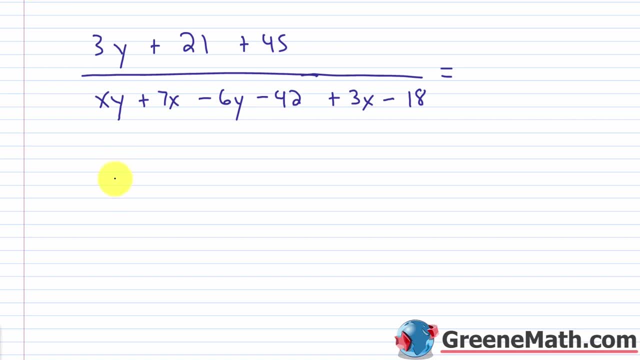 this would be 66. So this would be 3y plus 66 over in the denominator. what can I do? I have xy, I have 7x plus 3x, which is 10x, so plus 10x. 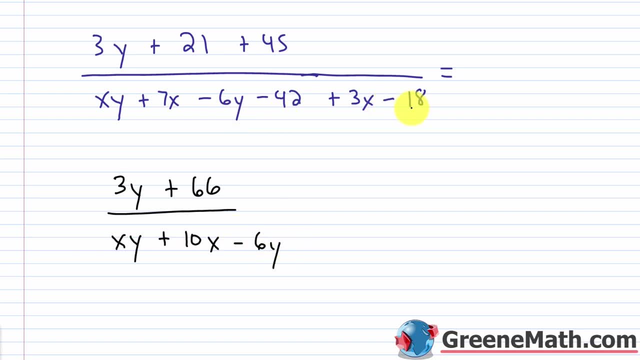 I have negative 6y, and then I have negative 42 minus 18,, which is minus 60. So the question is: can I factor anything and cancel? Well, I know in the numerator I could factor out a 3.. 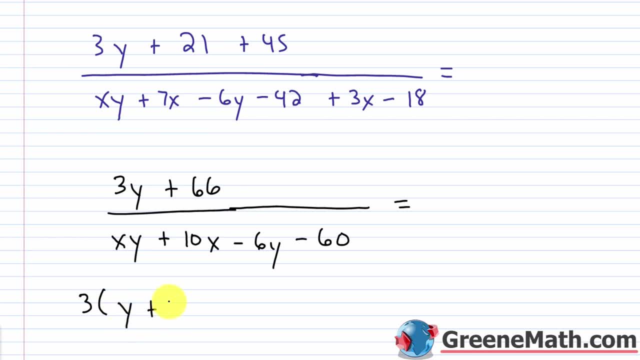 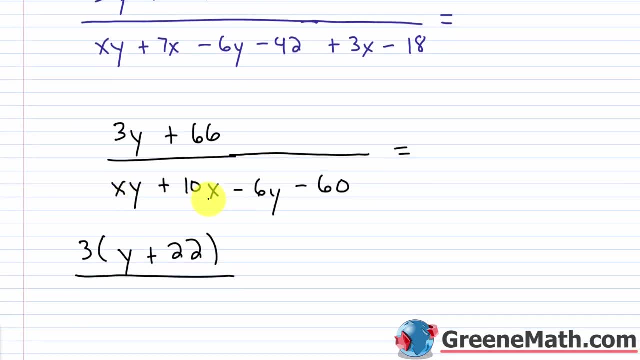 So I could factor out a 3, and I would have y plus 22,. okay, In the denominator could I factor that using grouping? Well, in the first group I could pull out an x. that would leave me with y plus 10.. 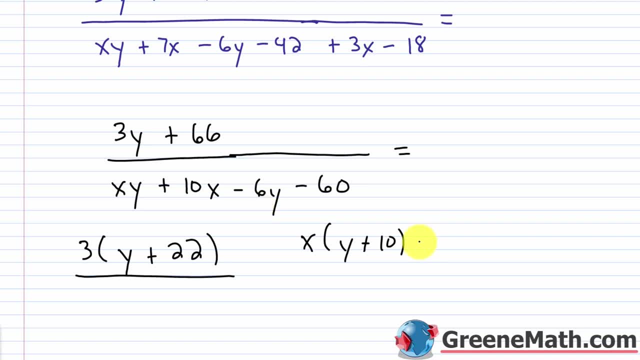 In the second group, I could pull out a negative 6, that would leave me with what A? y plus 10.. So if I factor out that common binomial factor, I would have the quantity y plus 10 multiplied by the quantity x minus 6.. 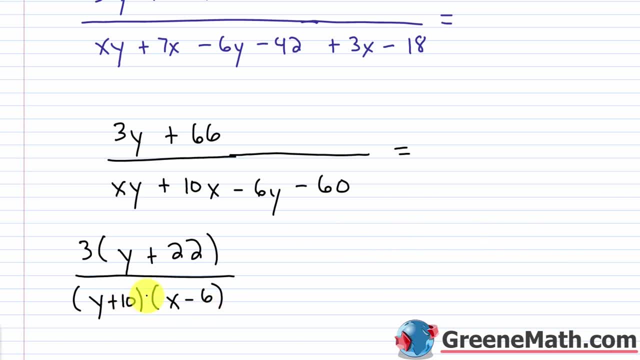 So it does factor, but it just doesn't do me any good. I can't do anything with it. I have a 3, nothing to cancel with. I have the quantity y plus 22,, nothing to cancel with. So I just leave it in factored form. 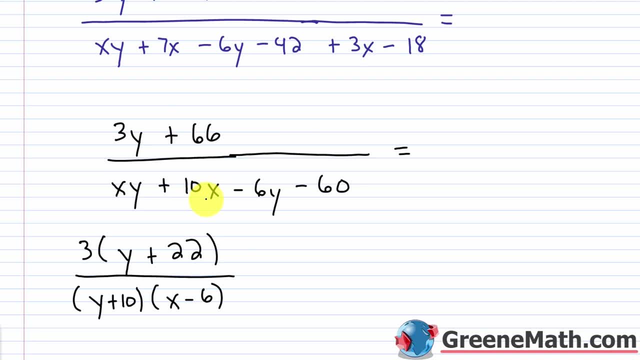 You could report your answer this way, but you're kind of leaving it open to yourself. hey, could I have factored stuff? So you want to just leave it in factored form to say, hey, there's no way that I could have. 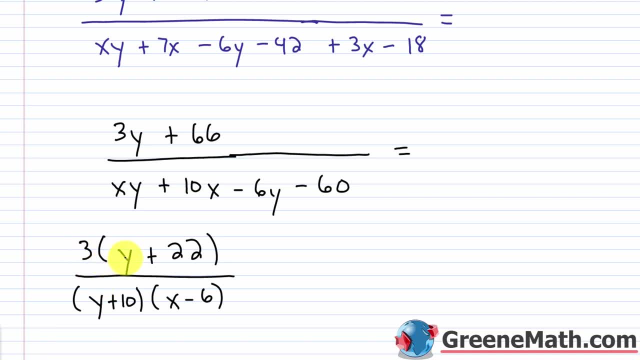 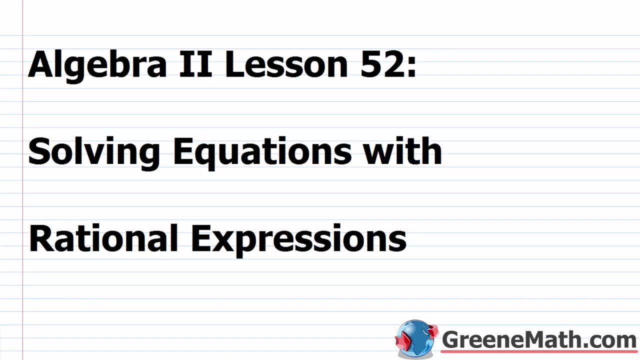 canceled anything. See here's the proof. So 3 times the quantity y plus 22 over y plus 10, that quantity times the quantity x minus 6.. Hello and welcome to Algebra 2 Literature. Let's get started. 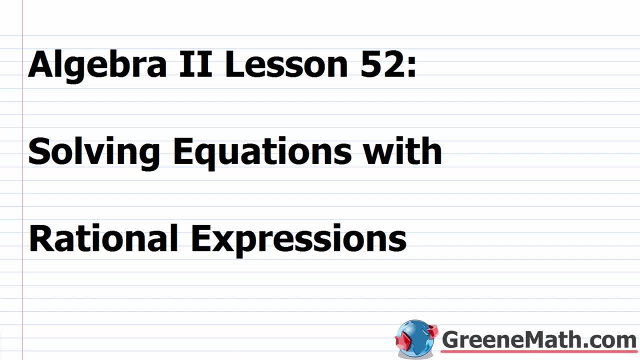 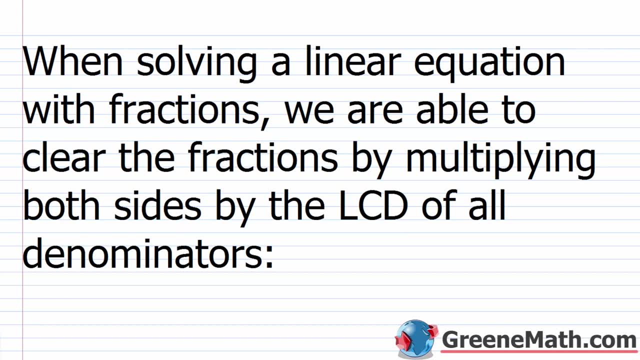 This is Lesson 52. In this video we're going to learn about solving equations with rational expressions. So again we've come to a subject that is something we learned back in Algebra 1, but we want to review in Algebra 2 to make sure we completely understand it. 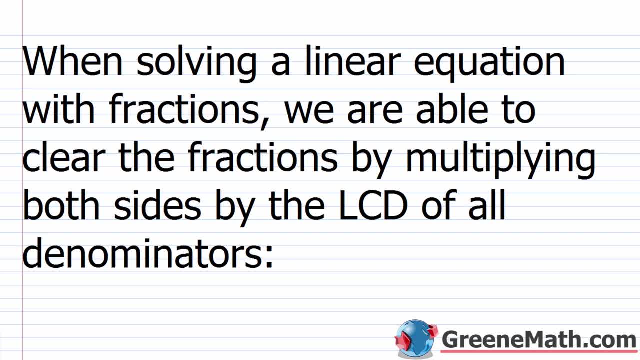 And that's so that when we get to tougher material we just have a better foundation. We'd rather see something twice and completely understand it, versus once and just kind of halfway understand it. So I want to start by just jogging your memory a little bit and I want to talk to you a 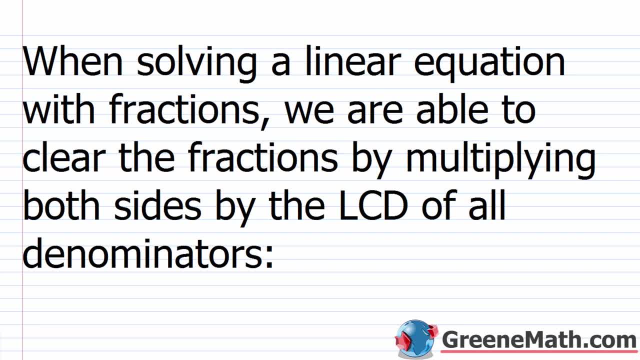 little bit about how we solve linear equations with fractions. So when solving a linear equation with fractions, remember, we are able to clear the fractions by multiplying both sides by the LCD, again the least common denominator of all denominators involved. So again, we saw this at the beginning of Algebra 2, when we reviewed our topic of solving. 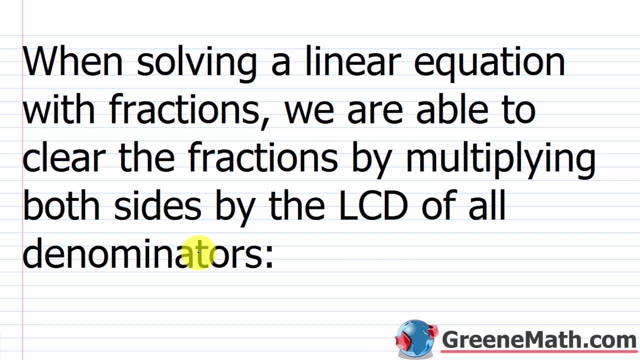 linear equations in one variable. I believe there's several of those in this paper, So why with 2?? It's select within Same between Three questions in depth in Algebra 1.. We spent a lot of time on that But I just 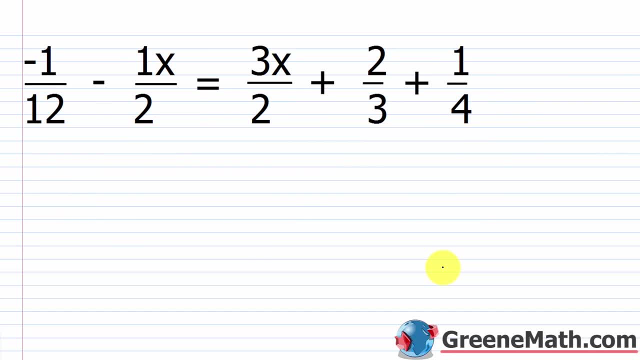 want to go through and look at a quick sample problem And I want you to look at this and try it on your own. So you have negative 1 twelfth minus 1 half x is equal to 3 halves x plus 2 thirds plus 1 fourth. So obviously, if you get something like 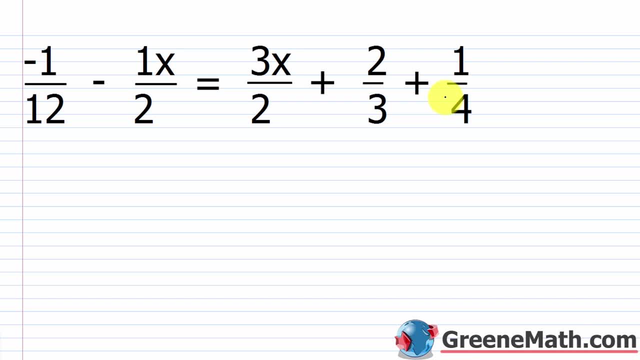 this you are able to work with the fractions. You can go through and do the same process just working with fractions, But it's usually going to be easier to multiply both sides by the LCD and just clear the fractions. So if I look at all the denominators involved, I have a 12,. 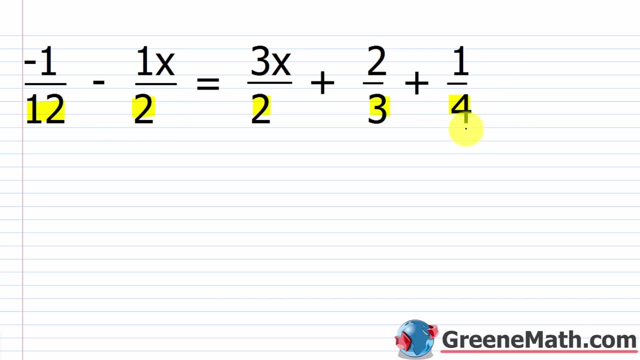 a 2,, a 2,, a 3, and a 4.. Now, 2 and 3 are prime numbers. 12 is what It's, 4, which is 2 times 2, and then times 3.. 4, I'm going to write as 2 times 2.. 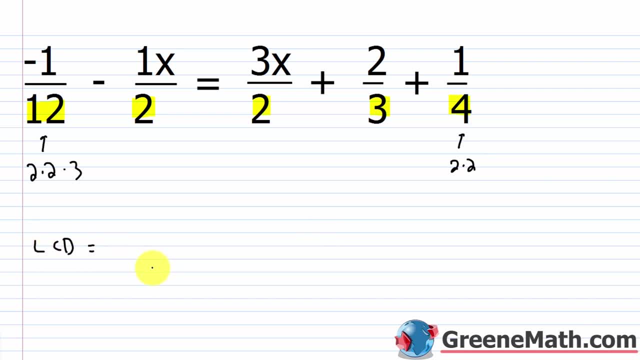 So when I build my LCD, what's going to go in there? Well, again, it's the largest number of repeats if I have something that's duplicated. So I have 1, 2 here, 1, 2 here, 2, 2s and 2, 2s- The largest number. 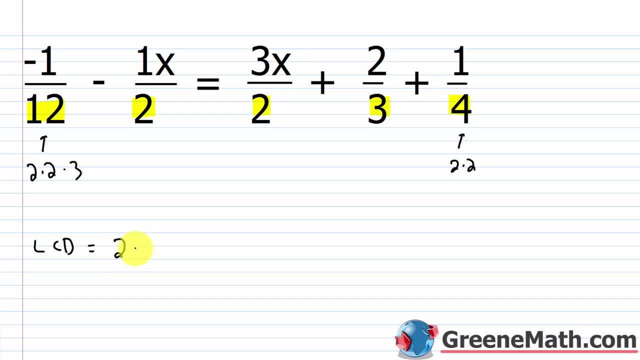 of repeats is 2.. So when I build my LCD it's going to be 2 times 2.. And then the only other prime factor I have: I have a 3 here, 1 occurrence, and I have a 3 here, 1 occurrence, So I'm just going to throw. 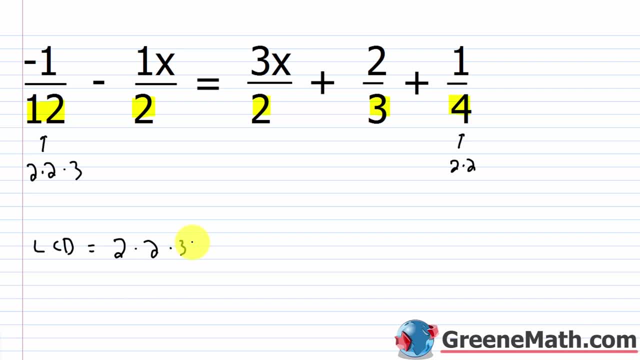 one of those in and my LCD is what It's: 2 times 2,, which is 4 times 3,, which is 12.. So I would multiply both sides of this equation by 12.. Very easy to do, And so let's set that up. We'd have 12 times the quantity You have. 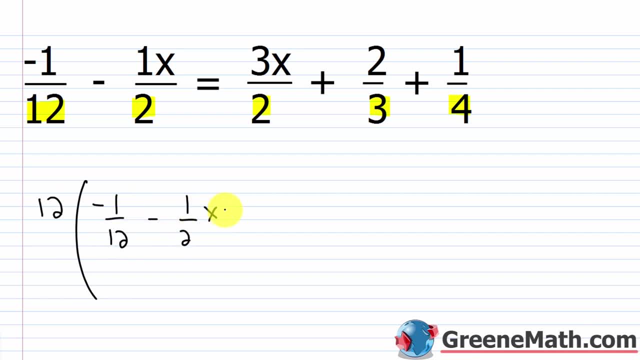 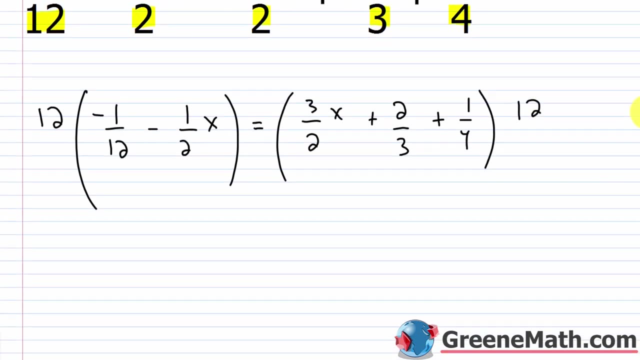 negative 1. twelfth minus 1 half x, and then this is equal to put parentheses around the other side, you have 3 halves x plus 2 thirds plus 1 fourth. Again, I'm multiplying this side by 12 as well. So what are we going to have here? 12 times negative 1. 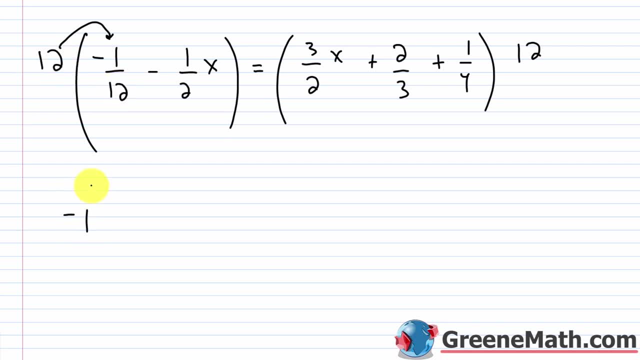 twelfth, We know the 12, we cancel the 12, I get negative 1.. Then 12 times negative 1, half x 12, we cancel with 2 and give me 6.. So I'd have minus 6x. So this equals. 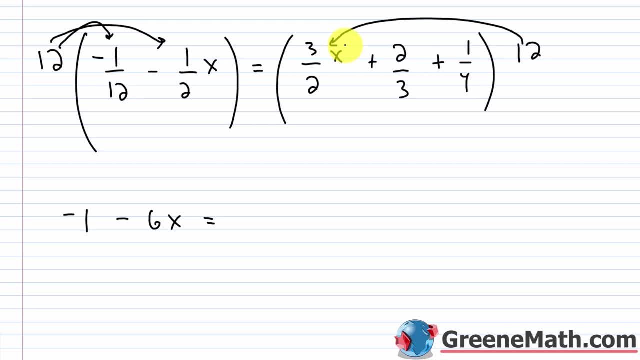 so I've got to do the same thing over here. 12 is going to multiply by 3, halves x 12, we cancel with 2 and give me 6.. 6 times 3 is 18, so I'd have. 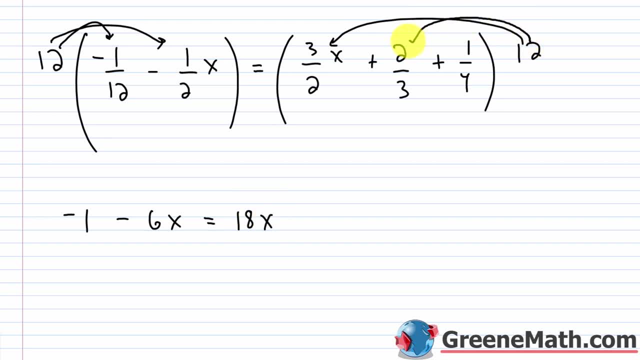 18x there And then here I'd have 12 times 2 thirds, So 12, we cancel with 3 and give me 4.. 4 times 2 is 8, so plus 8.. Then you'd have 12 times 1 fourth, 12, we cancel. 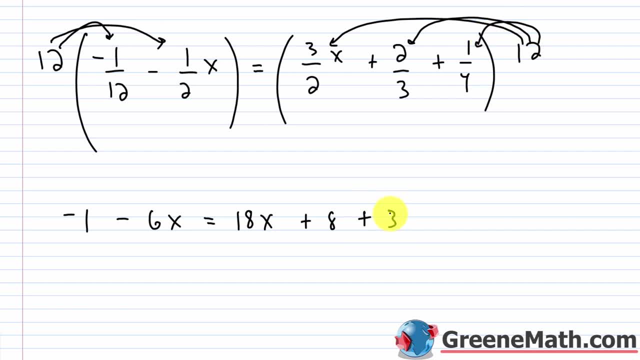 with 4 and give me 3.. So you'd have plus 3.. So now I would simplify this: 8 plus 3 is 11.. So let's just write 11 there, And I can't really do anything else on the left or the right. So I'm going to move all my variable terms to the left. 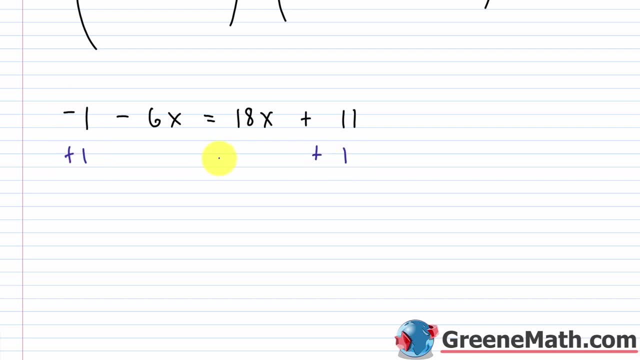 all my numbers to the right. So let me add 1 to both sides And let me subtract 18x from both sides, So this will cancel, and this will cancel Negative 6x minus 18x is negative 24x And then 11 plus. 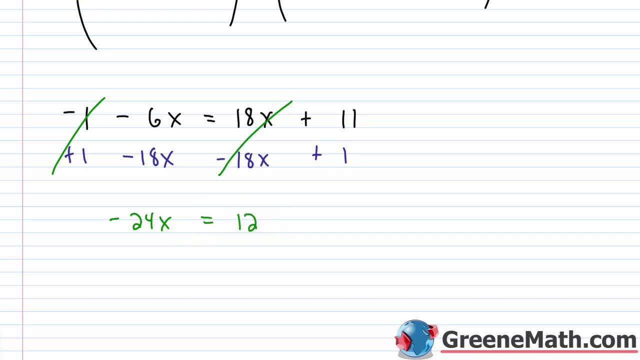 1 is 12.. So this equals 12.. Let's go ahead and divide both sides of the equation by negative 24.. So what's going to happen is this will cancel with this and just give me x, And this will be equal to: you've got 12 over negative. 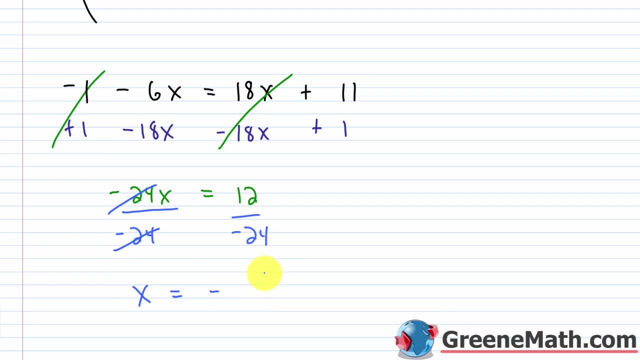 24.. So I know it's negative. And then 12 over 24 is going to be what? That's 1 half. So this is negative 1 half. Now you can check this. if you want, You can pause the video and go back. I can assure you, I've checked and it does work. 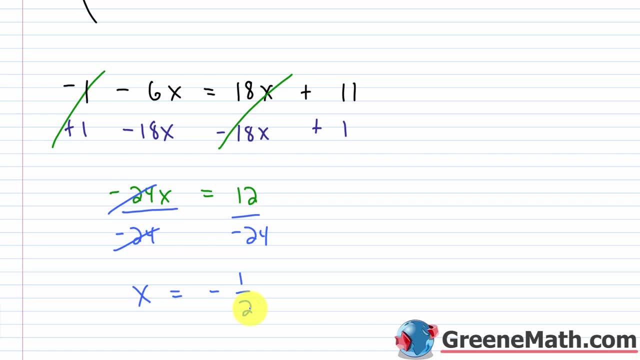 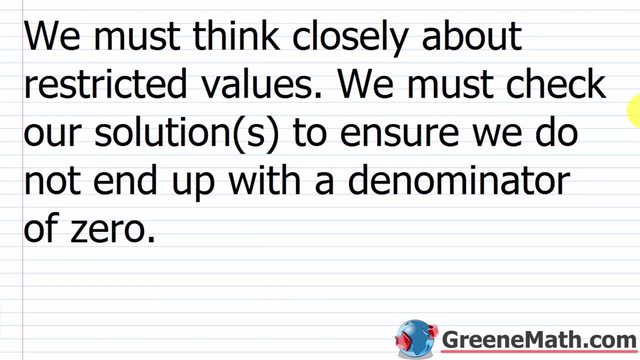 But essentially I'm just jogging your memory on how you go about doing these things. You want to multiply both sides by the LCD so you can clear the fractions, All right. so now that we've kind of thought about this a little bit, I want you to think about applying the same technique if you had an. 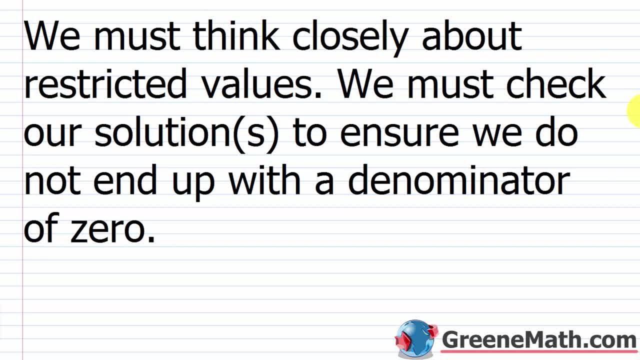 equation with rational expressions, The main thing you have to be careful about: we must think closely about restricted values. So let me highlight that. Remember we talked about restricted values at the beginning of the chapter where we started talking about rational expressions. in general, We have to check solutions to ensure we do not end up with a denominator of zero. 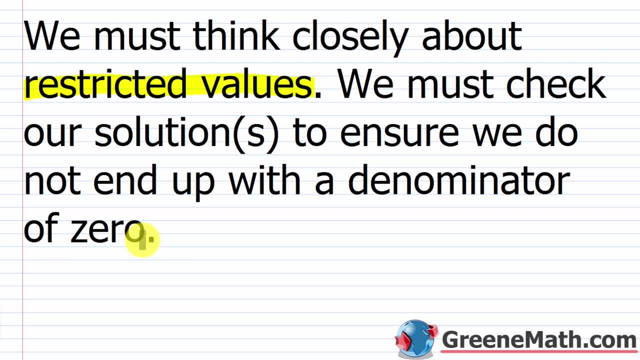 Remember we can never divide by zero. So if you get x equals some value and when you plug it in it gives you a denominator of zero, you have to reject that solution. That solution is not valid. Let's just take a look at the first problem. We're going to start out with a very easy one here. 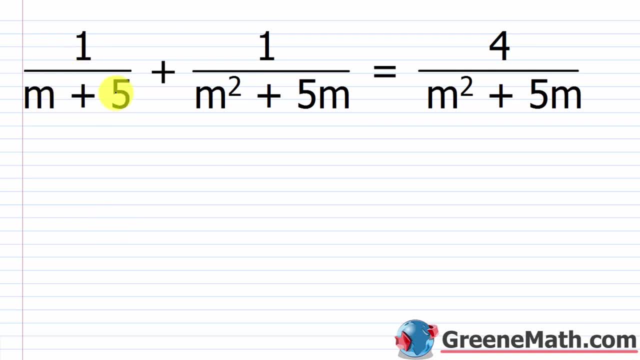 just to kind of get our feet wet. So we have 1 over m plus 5, plus 1 over m squared plus 5m, and this equals 4 over m squared plus 5m. So the first thing you always want to do is you want to. 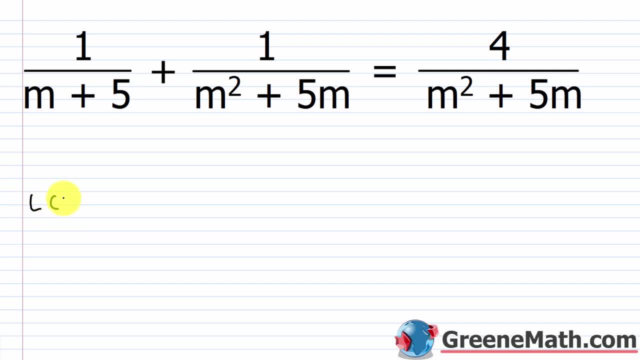 find your LCD. Sometimes the LCD is very easy to find. Other times it takes quite a bit of work because of the amount of factoring you have to do. But for this one it's very, very easy. m plus 5 doesn't factor, So this is just m plus 5.. This guy and this guy are the same, We know. 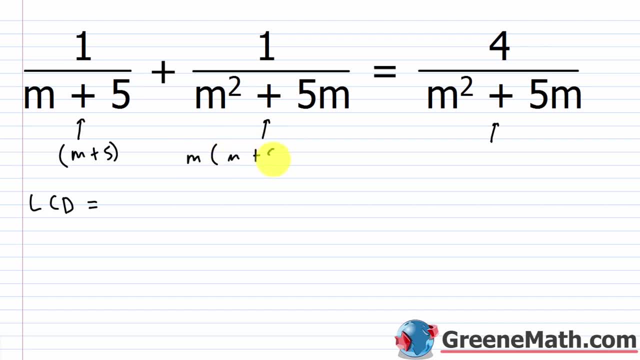 that that would factor into what m times the quantity m plus 5.. So a lot of you can already know that the LCD is just m times the quantity m plus 5.. When you build the LCD again you look at your factors. Every factor would go in there, but if there's a duplicate right or something that's 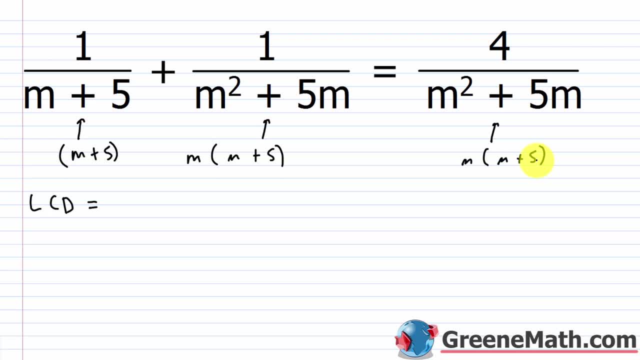 common to more than one of these, then what you're going to do is you're going to go with the largest number of repeats. Well, I've got 1 m plus 5 here, 1 here and 1 here, So I would 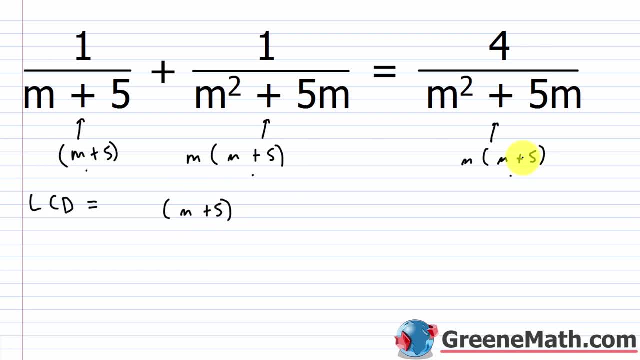 just throw 1 in when I build my LCD. Then you look at m, m occurs here and here only occurs once in each. So I only put 1 in when I'm building my LCD. So the LCD or you can also. 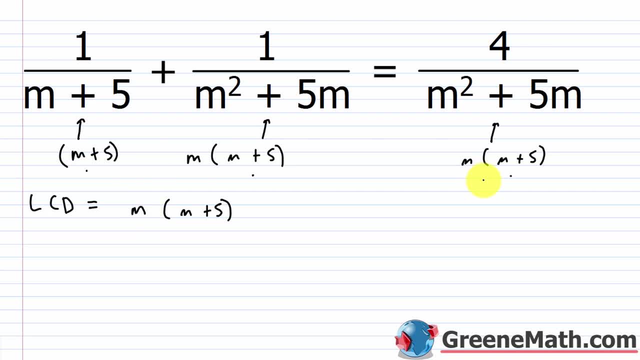 say the LCM. right, the least common multiple of these guys is going to be m times the quantity m plus 5.. So that's your least common denominator, or your least common multiple of these denominators. Okay, So now that we know that, the next step is very, very easy. We're just going to multiply. 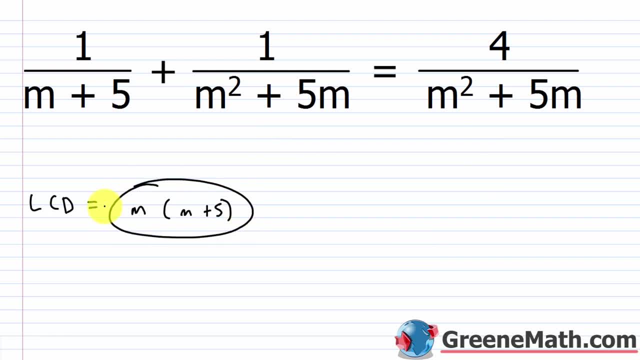 this right here, just like we did with that example where we cleared the equation of the fractions: m times the quantity m plus 5 is going to be multiplied by 1 over m plus 5.. And then plus this is going to be multiplied by that, So 1 over m times the quantity m plus 5.. 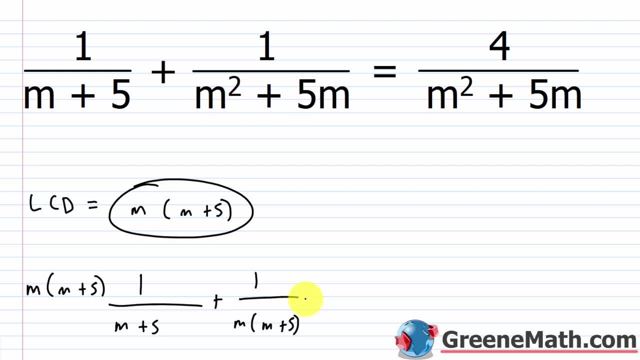 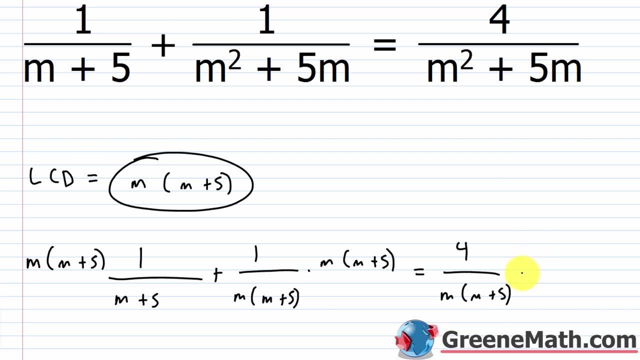 And that's just this in factor form. All I did was factor out an m, So times we're going to have m times the quantity m plus 5.. And this equals you've got a 4 over m times the quantity m plus 5.. Again, I just factored that, That's all I did. Times you have m times the quantity m plus. 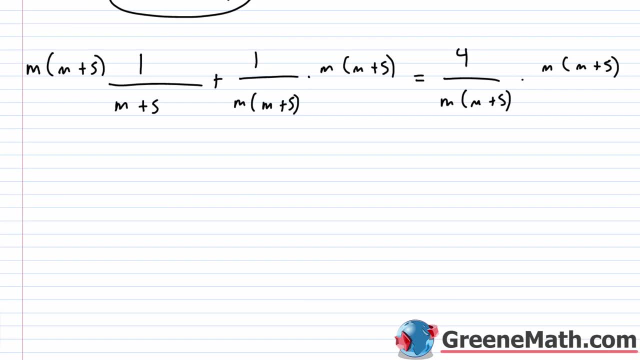 5. So super easy example. What you're going to see is that when you multiply here, this would cancel with this. You'd have m times 1 or just m, Then plus. The next thing is this cancels completely with this. So I would have m times 1 or just m, And then plus, And then plus, And then. 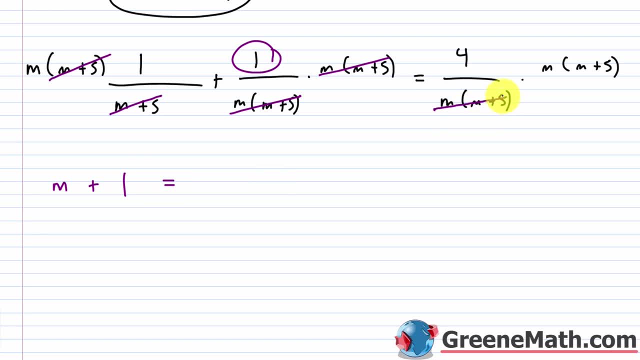 I would just have a 1.. Then this equals Over here. this cancels completely with this, So I would just have a 4.. So m plus 1 equals 4 is about as simple as it gets in terms of solving equations. We just subtract 1 away from each side And you get m is equal to 3.. So let's write that. 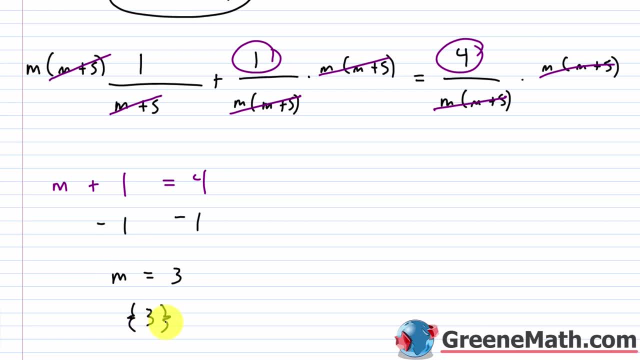 using a solution set also. We get some practice with that And you want to go back and you want to check for two things. The first thing would be make sure the left and the right side is equal. You could get an answer that doesn't make your denominator 0, but it might not still work. The 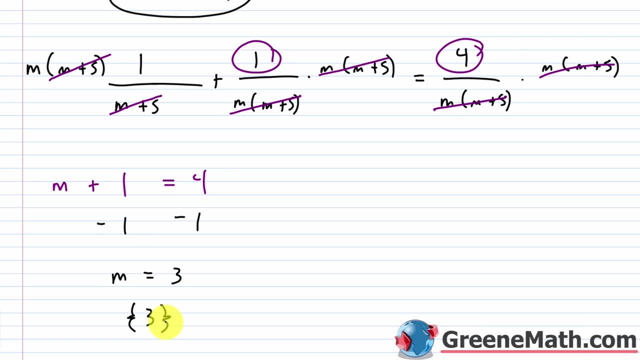 other thing is you got to make sure that your answer or your solution does not result in a denominator that's 0. If you get that, you've got to reject that solution. It's not valid. So let's go back up. Let me just erase everything here And I'm going to plug in a 3. Everywhere. 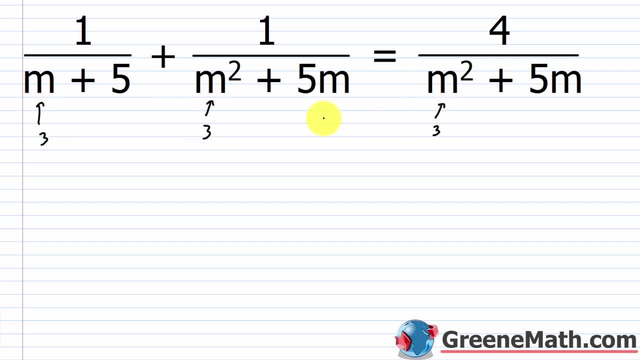 there's an m And let's see what we get. So we'd have m times m plus 4.. And then plus, And then we'd have 1 over 3 plus 5.. 3 plus 5 is 8.. So this would be 1 eighth plus. You'd have 1 over 3. 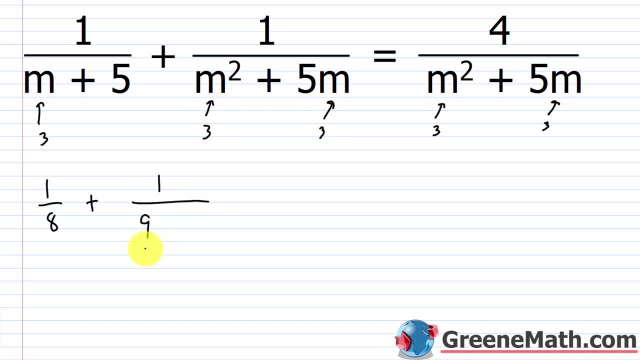 squared is 9.. 5 times 3 is 15.. 15 plus 9 would be 24.. This should be equal to. we have 4 over 3. squared is again 9 plus 5 times 3 is 15.. So again, this would be 24.. Now you don't need to. 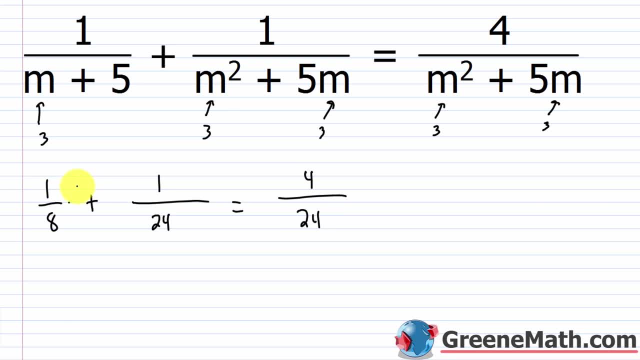 reduce this fraction. All you want to do is get a common denominator over here. So multiply this by 3 over 3. And you would get what You would get. 3 24ths plus 1 24th is equal to 4 24ths. 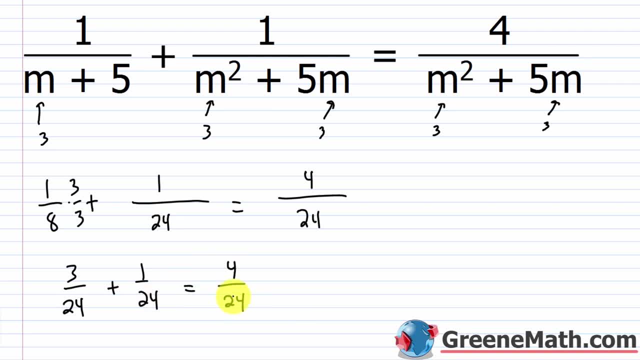 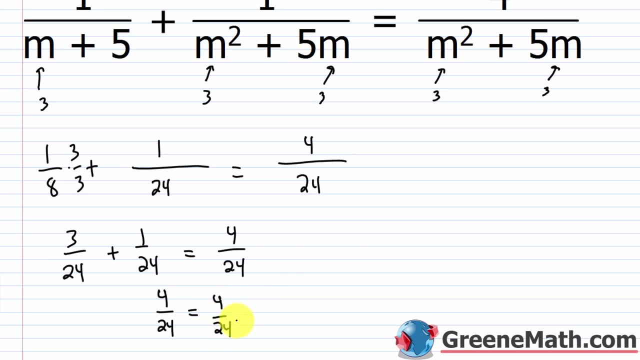 Well, yeah, that checks out. 3 plus 1 is 4.. 4 over 24 is 4 24ths. So you would get: 4 24ths is equal to 4 24ths. And then, if you want to, after you've done that, you can go ahead and 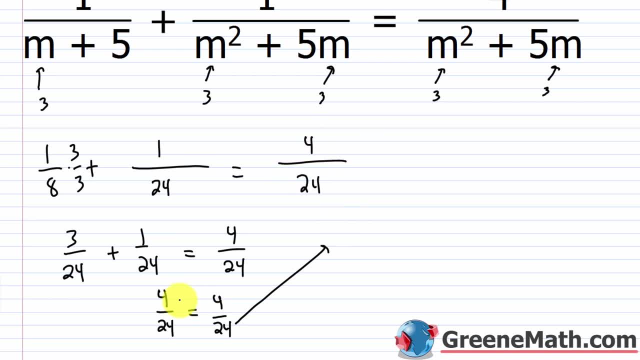 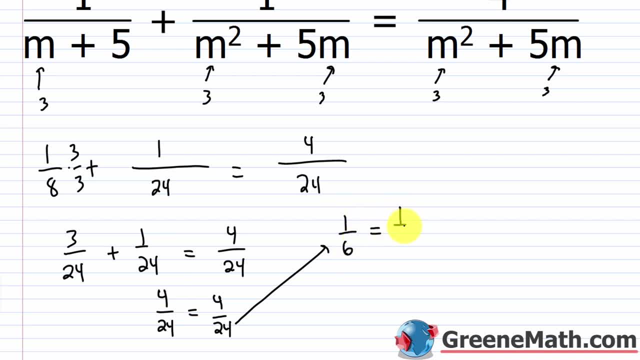 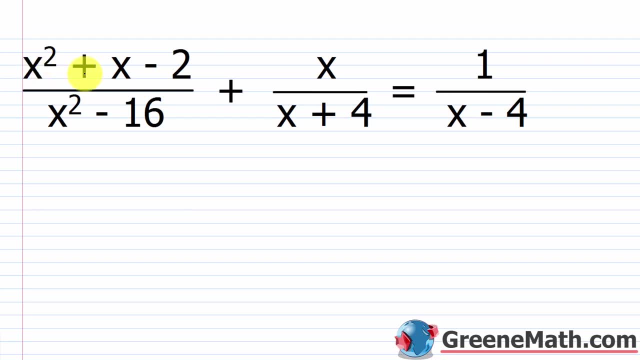 by 4 is 1.. So this would be 1: 6 is equal to 1, 6.. All right, so let's turn up the heat just a little bit And we'll look at one that's a little bit more challenging. So we have x squared plus. 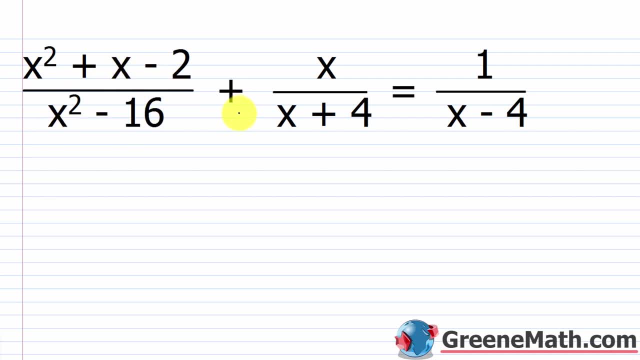 x minus 2 over x, squared minus 16.. Plus we have x over x plus 4. And it equals 1 over x minus 4.. So again, a lot of you who have done this before can already tell what the LCD is. 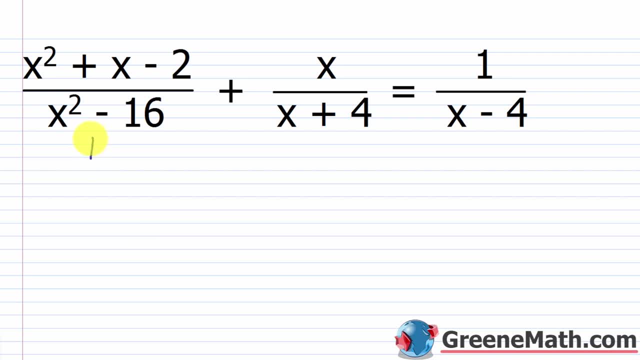 A lot of these problems kind of set up the same way. So this factors into what This is: x plus 4.. Times: x minus 4.. All right, this is the difference of two squares. Again you see a two-term polynomial with a minus. You got to be thinking the difference of two squares. Then you have x. 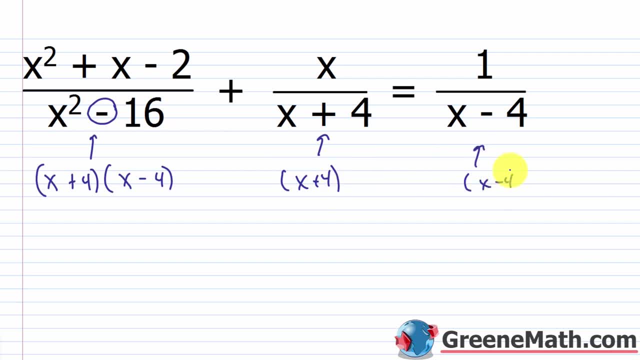 plus 4.. And then you have x minus 4.. So the LCD is what It's: x plus 4, that quantity times x minus 4.. So what I'd do is I would multiply both sides of the equation by that. So what I'm going? 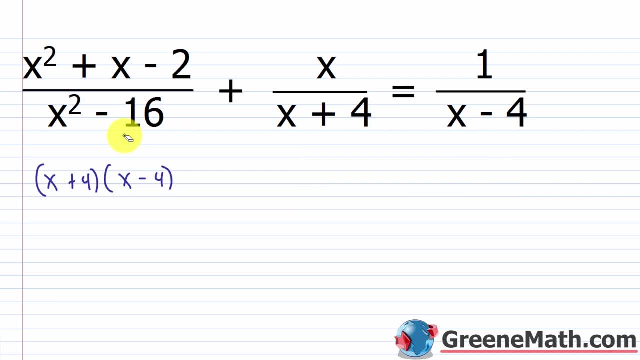 to do, because it's hard to fit this on the screen. let's just go through and, piece by piece, multiply. So if I multiply this times this, we know this would cancel- right- Because that is in factored form- the quantity x plus 4 times the quantity x minus 4.. So what would happen is I: 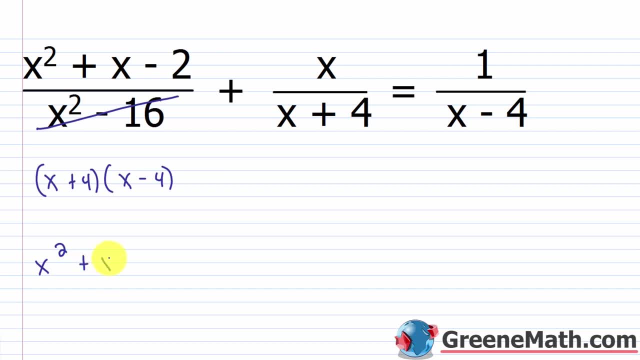 would just be left with the numerator, which is x squared plus x minus 2.. Now if I multiply this by this, the x plus 4 would cancel with the x plus 4. And I'd have x minus 4 times x, So you'd. 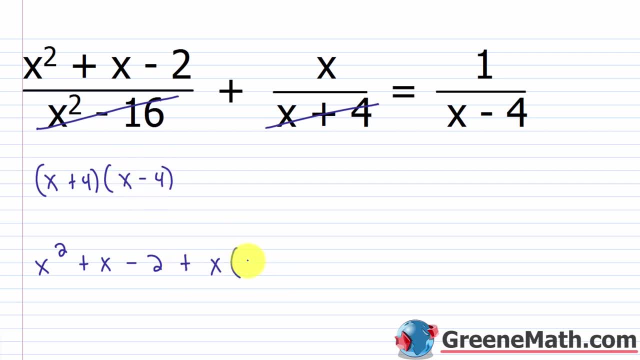 put plus and x out in front. Make sure this is in parentheses. Then equals: If I multiply this times this, the x minus 4 would cancel. You'd have 1 times the quantity x plus 4.. So you can put that in parentheses or not put it in parentheses. 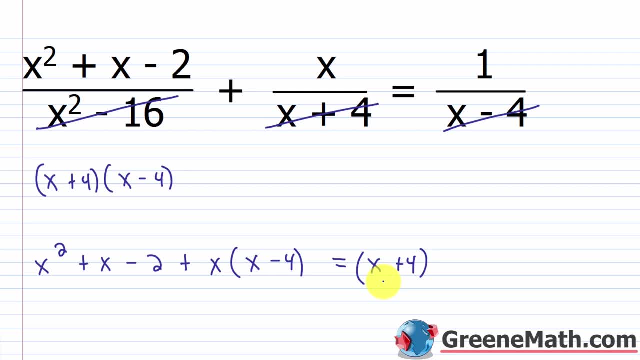 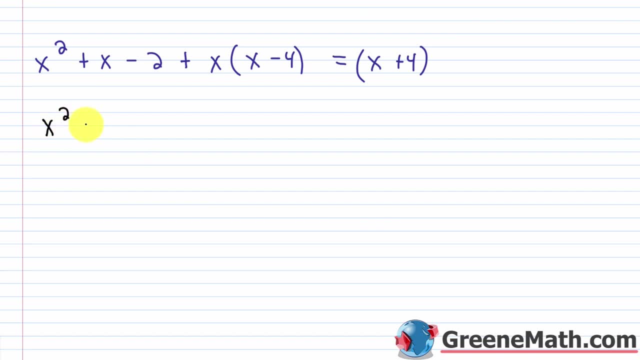 There's really nothing else over there, so it wouldn't matter, All right. So now that we have that done, let's just go through and simplify. So we'll have x squared plus x minus 2.. Then we have x times x, which is x squared. So we'll have x squared plus x minus 2.. Then we have x times x. 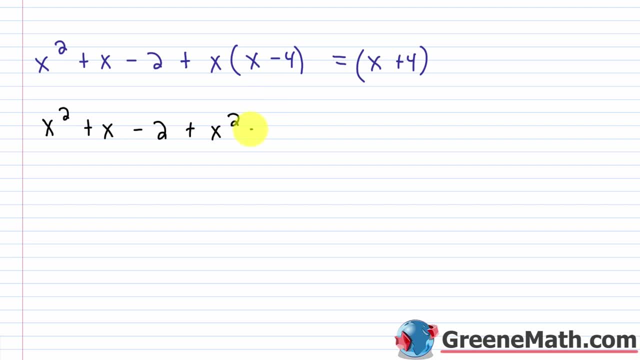 which is x squared. So we'll have x squared plus x minus 2.. Then we have x squared plus x minus 2.. Then we have x squared, so plus x squared, We have x times negative 4, which is minus 4x. 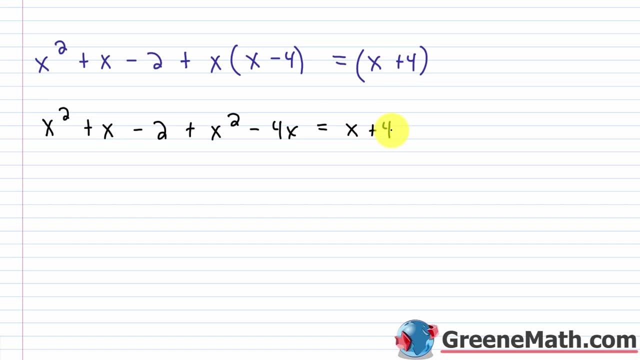 This equals again we have x plus 4.. So what I can do again, if I see that I have x and x on two different sides of an equation, I can get rid of that right, Because if I subtracted x away, 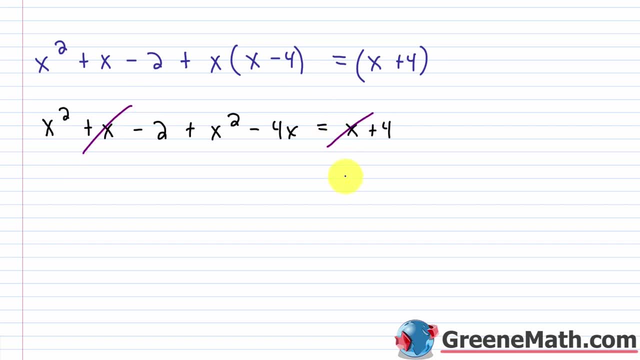 from each side, this would go away. So then what else can I do? On the left side, x squared plus x squared is 2x squared, Then we have minus 4x, so minus 4x, Then we have minus 2x and this equals 4x. So we're going to be dealing with a quadratic equation. 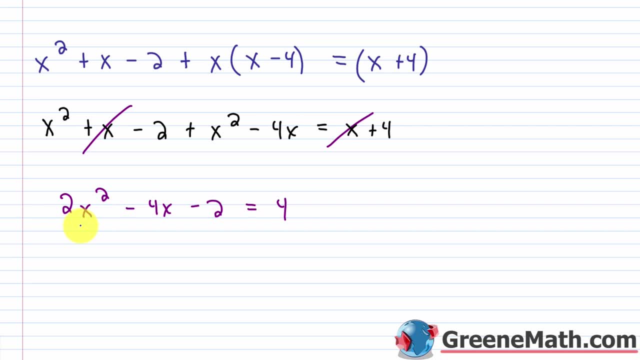 And I know we talked about the quadratic formula back in Algebra 1.. We have yet to review it in Algebra 2.. So I just gave you something you could factor right So we could solve this using the zero product property. So let's subtract 4 away from each side of the equation. So this on this. 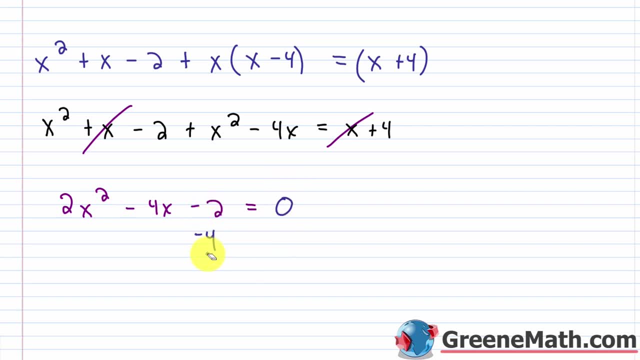 side would now be 0.. And over here, negative 2 minus 4 would be negative 6.. So let's factor this guy. So the first thing you'd notice here is: you can pull a 2 out. You'd be left with x squared minus 2x minus 3.. 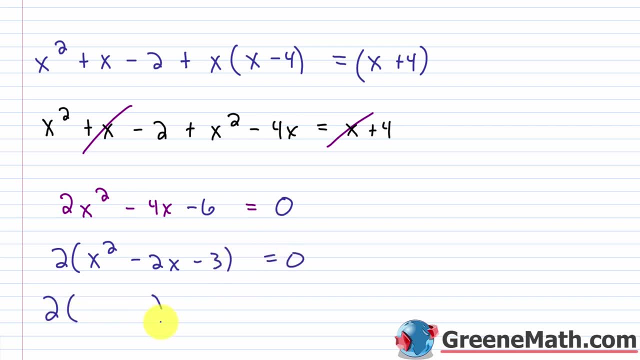 This equals 0.. Of course, the 2 would still be out in front. You set this as a product of two binomials, So you'd have x here and x here And just give me two integers whose sum is negative 2. 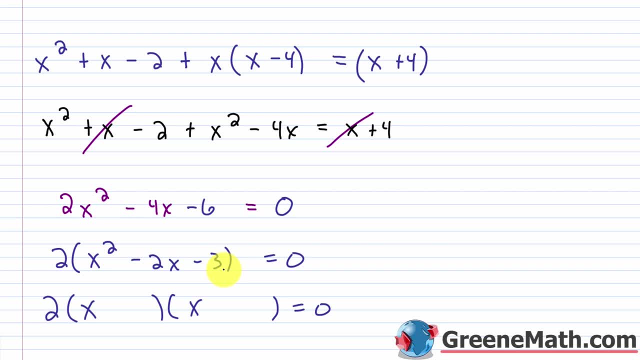 and whose product is negative 3.. Well, you could go with negative 3 and positive 1.. So minus 3 and positive 1.. Negative 3 times 1 is negative 3 and negative 3 plus 1 is negative 2. So that would work. 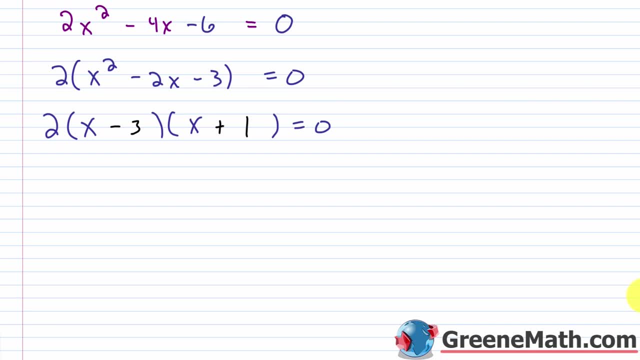 So, to solve this now, what we're going to do, we're going to take each factor with a variable. So this factor here and this factor here, We're going to set them equal to 0 and we're going to solve. So you would have: x minus 3 is equal to 0. 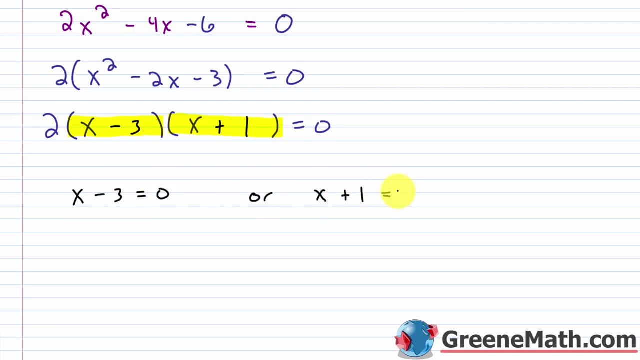 or x plus 1 could be equal to 0.. You add 3 to both sides of the equation here you get x equals 3.. Over on this side you subtract 1 away from each side of the equation. You get x is equal to negative 1.. 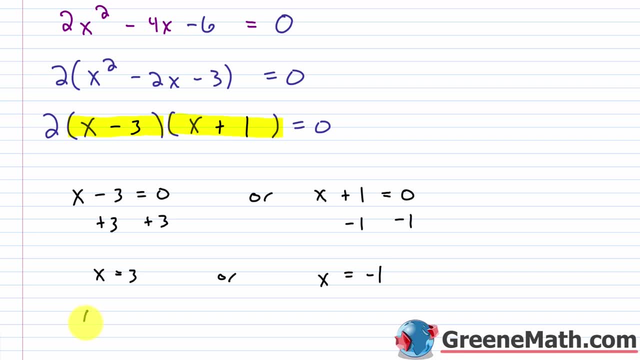 So my solution- or in this case would be solutions- would be what? x could be negative, 1 or it could be 3.. Now I put that as the solution set now, But I can't actually say that it's the solution until I check. 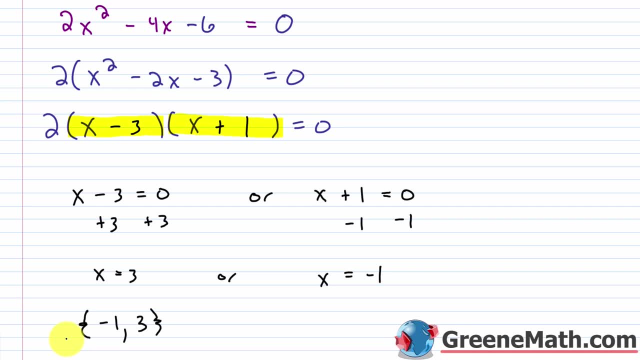 to make sure that it doesn't make the denomination, Or any denominator, equal to 0 in that rational expression. Now I've set up my solution, set here, but it might not be true Because, again, remember, I've got to check to make sure that no rational expression. 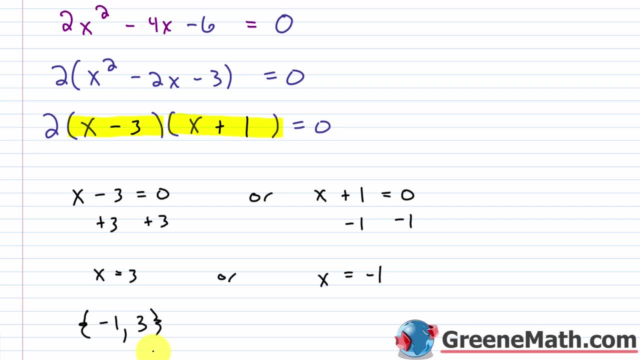 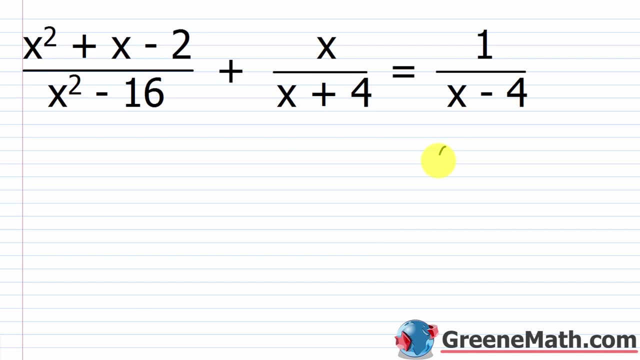 has a denominator of 0 when we substitute these values in for our variable x. So let's check that out real quick, Alright. so again, the proposed solutions were negative 1 and 3. So let's check negative 1 there. So I'd plug in a negative 1 there. 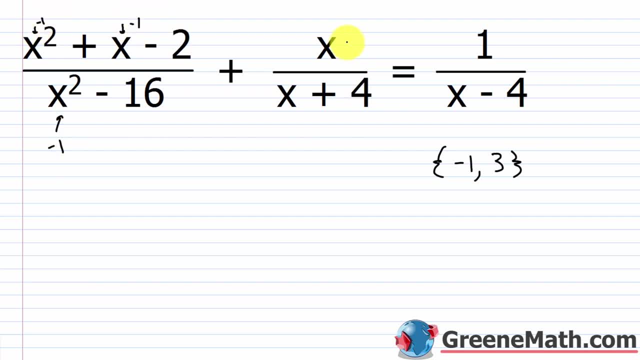 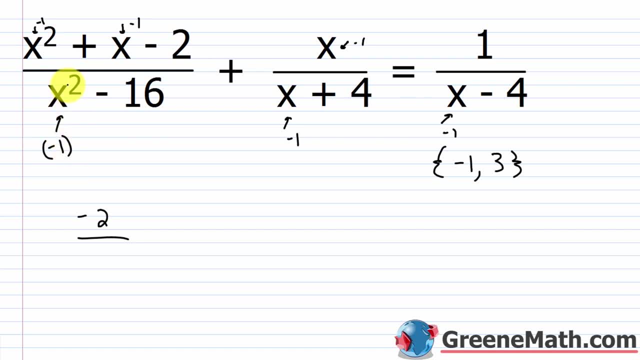 And the denominator negative 1 squared- and this would be in parentheses because I'm plugging in for the x. So negative 1 squared is 1.. 1 minus 16 is negative 15.. So this would basically be negative over negative. 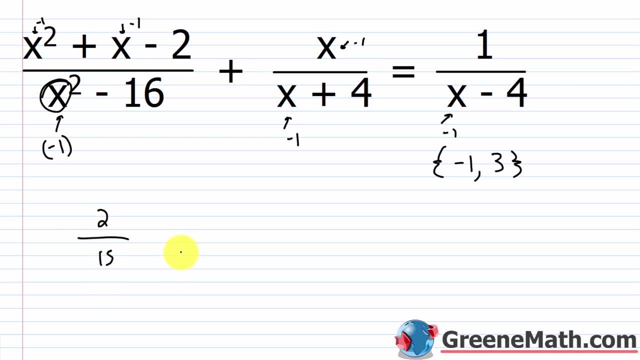 positive, So positive 2, 15ths. Then we have a negative 1, a negative 1, over you have negative 1 plus 4, which is positive 3. So you can put negative 1, third, there you can put plus, like that: 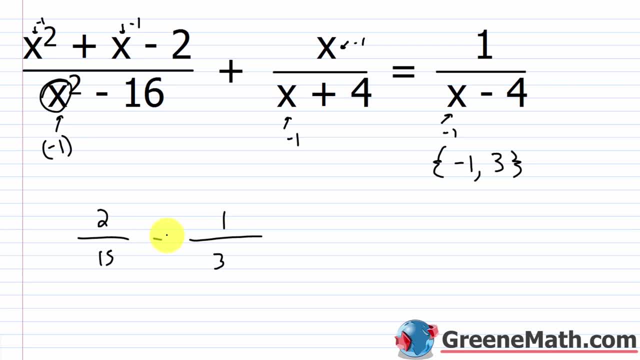 or you can just simply say it's minus 1 third. Whatever you want to do, Then this is going to be equal to: we have 1 over. you have negative 1 minus 4.. Negative 1 minus 4 is negative 5.. So you can say this is negative 1.. 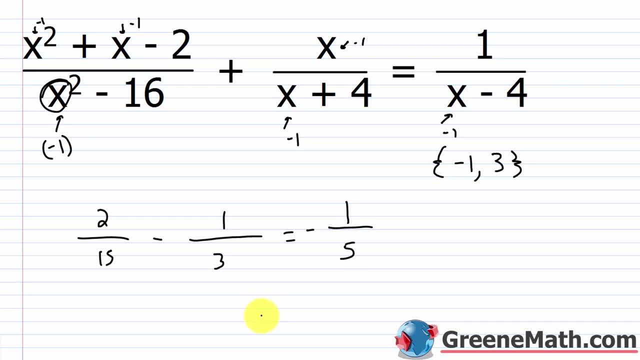 All right, So let's get a common denominator going here. If I multiply this by 5 over 5, what I'd have is 2 minus 5 over 15.. Now, 2 minus 5 is what That's negative 3.. 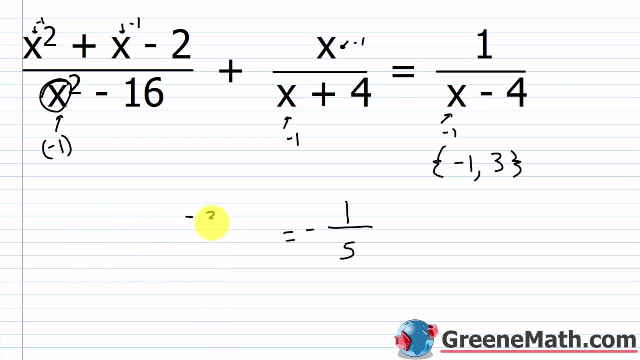 So you'd have negative 3 over 15, negative 3 over 15, which of course would simplify to negative 1 fifth. So you get negative 1 fifth equals negative 1 fifth. So this one checks out, Doesn't make any denominator zero. 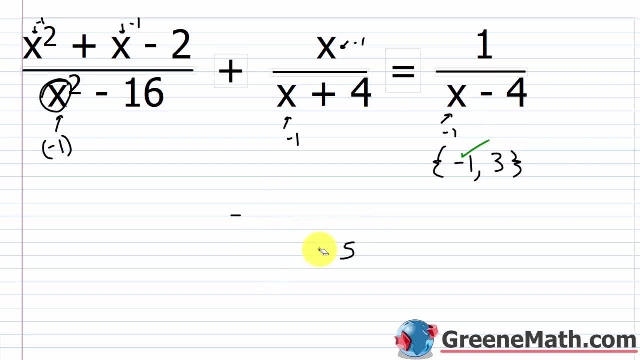 Left and right side are equal. Good to go on that. The next one we want to check is 3.. We want to check 3.. All right, So you'd have 3 squared, which is 9, plus 3 minus 2, over 3 squared again, which is 9 minus 16,. 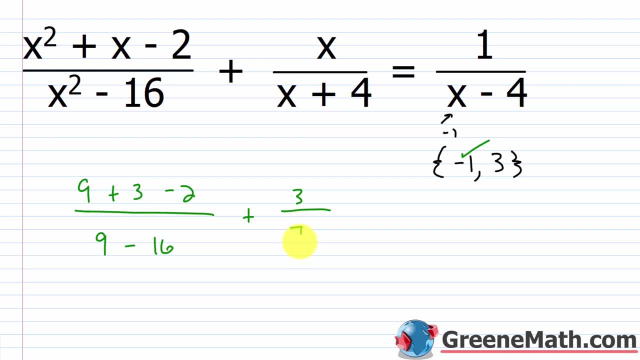 plus, you'd have 3 over 3 plus 4, which is 7.. This equals 1 over 3 minus 4,, which is negative 1.. So 1 over negative 1 is just negative 1.. Let's write that like that: 9 plus 3 is 12.. 12 minus 2 is 10.. 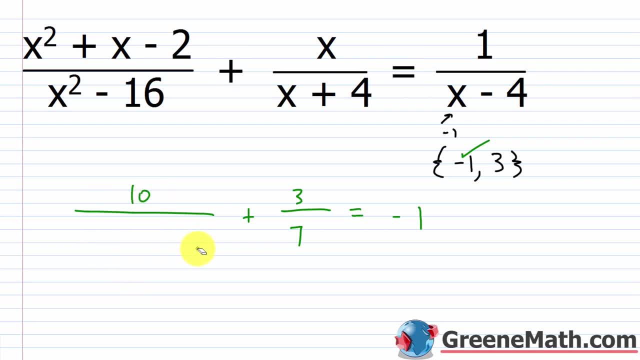 9 minus 16 is going to give me negative 7.. Now what you can do here you have a positive over a negative. I want a common denominator with this, So all I need to do is bring this negative into the numerator and erase it from the denominator. 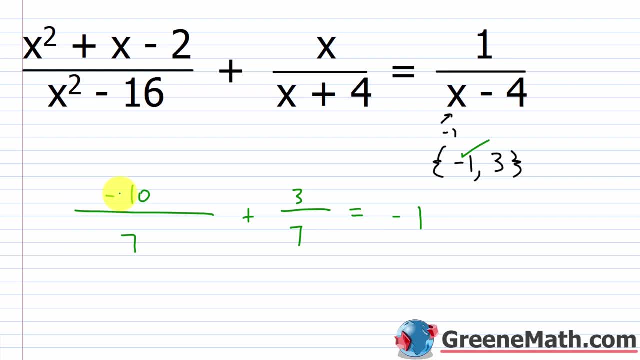 Negative 10 divided by positive 7. Is the same thing as 10 divided by negative 7.. So now I have negative 10 plus 3,, which would give me negative 7.. So this would be negative 7 over 7,, which is also negative 1.. 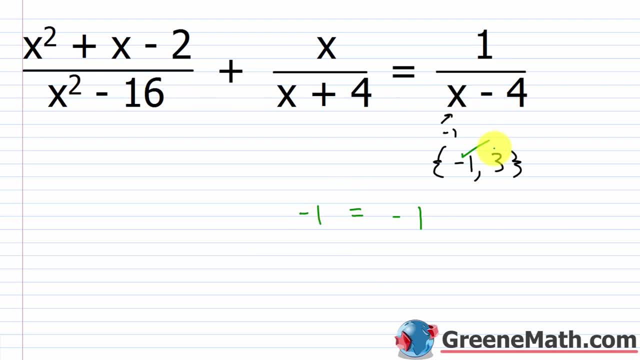 So the left and the right side are equal. None of my denominators became zero, So this works as a solution as well. So our solution set here contains two elements: negative 1 and 3.. Each one of those can be substituted in for x. 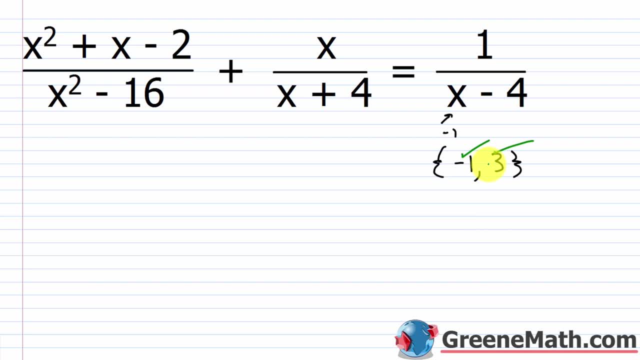 Again, no denominator becomes zero, And the left and the right side would be equal for each of them, So we get negative 7 over 7.. Now let's take a look at one final problem. This is going to be one that's going to be. 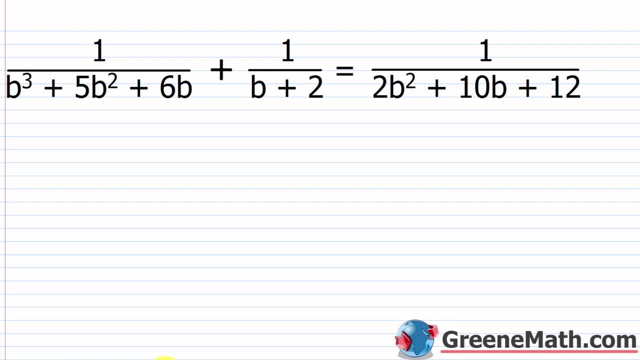 kind of tedious, kind of take a little bit of time, but it's typical when you get to Algebra 2 to get more tedious problems. So we have 1 over b cubed plus 5b squared plus 6b. Plus we have 1 over b plus 2. And this is equal to: we have 1 over 2b squared plus 10b plus 12.. 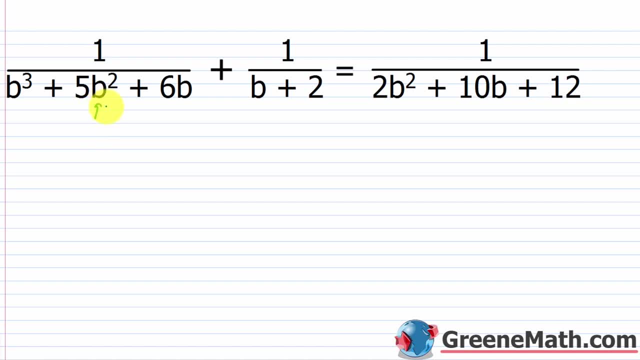 So obviously we want to get the LCD. So for this one I would start by just pulling out a, b. Now it would give me b squared plus 5b plus 6.. Then I would say: okay, well, give me two integers whose sum is 5 and whose product is 6.. 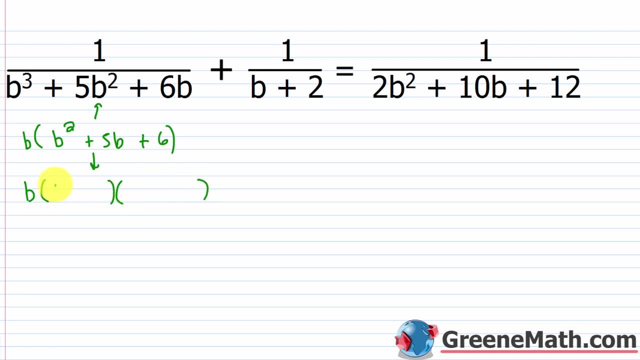 So we'd have b times and inside of parentheses I'd have b here and b here And to answer that question, the numbers would be 2 and 3.. Right, So if I had positive 2 times positive 3, I'd get 6.. Positive 2 plus positive 3 would give me 5.. So b plus 2 and b plus 2.. So b plus 2 and b plus 3.. So if I had positive 2 times positive 3, I'd get 6. Positive 2 plus positive 3 would give me 5.. So b plus 2 and b plus 2.. 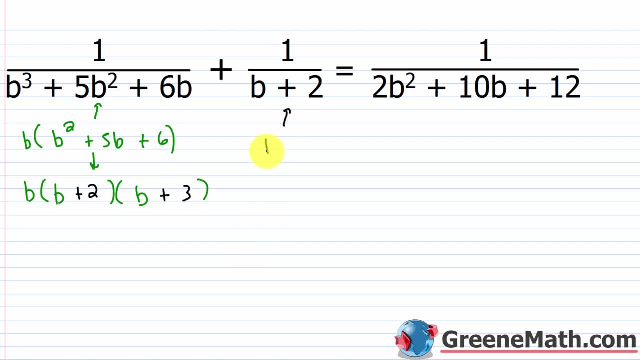 Now this guy right here is just b plus 2.. I can't factor that at all. So that's just what it is Over here, for the 2b squared plus 10b plus 12,, we could factor out a, 2, and we'd be left with b. 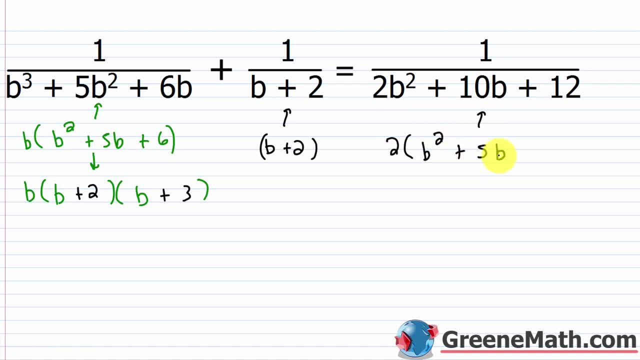 squared plus 5b plus 6.. Now, what do we notice from that? This is the same thing as this. So what we can do is say this is 2 times and just copy this: b plus 2 times, b plus 3.. 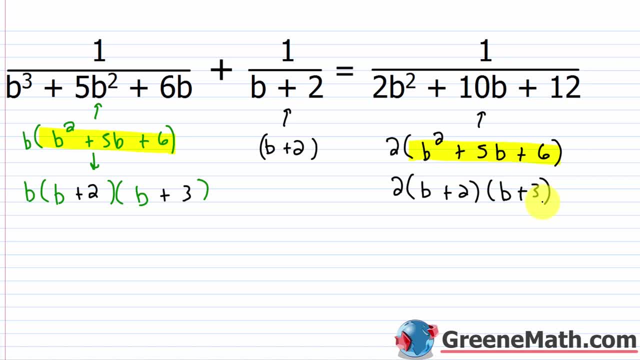 So what's our LCD going to be? Well, the LCD would what It would contain: one copy of b plus 2.. I've got b plus 2 here, here and here, So just one of those when I build the LCD. 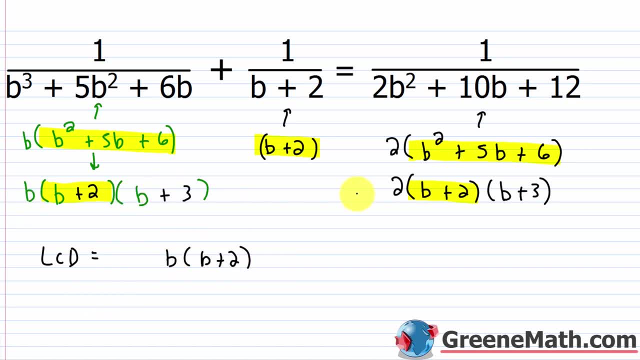 Then I've got a b, So let's put that out in front. I don't have that anywhere else, so I'm going to put that in. Then we have b plus 3.. So just one of those. So b plus 3 is going in. 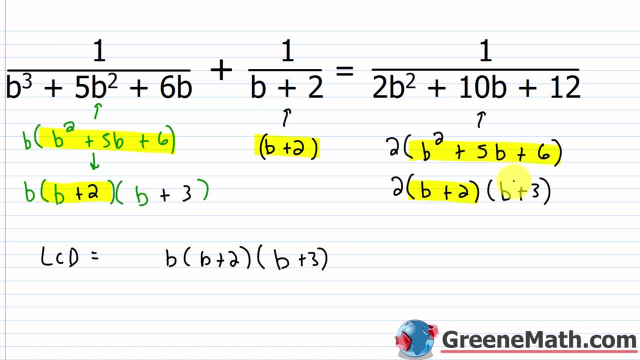 because it's here and here and it only occurs once in each, And then we also have a 2. So let's put that out in front. So the LCD is 2b times the quantity b plus 2 times the quantity b plus 3.. 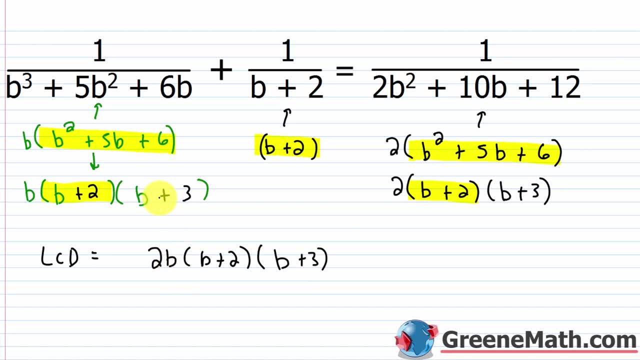 All right. So if I was to multiply the LCD by this first guy right here, what would cancel? Remember: in factored form, this is b times the quantity b plus 2 times the quantity b plus 2.. So if I were to multiply the LCD by this first guy right here, 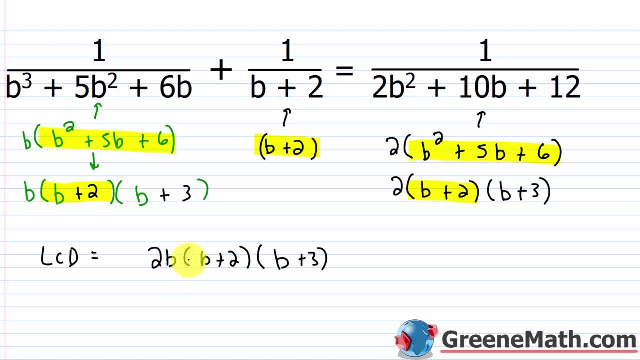 quantity b plus 3.. Here I have 2 times b times the quantity b plus 2 times the quantity b plus 3. So everything in the denominator would cancel and I would just be left with a 2 times this 1,. 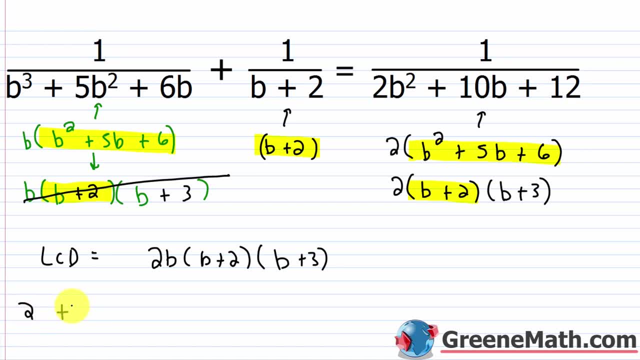 which would give me 2.. Then you'd have plus. If I multiplied this times this, the b plus 2 would cancel. so this would be gone. What would happen is I'd have 2b times the quantity b plus 3 times 1.. So 2b times the quantity b plus 3.. 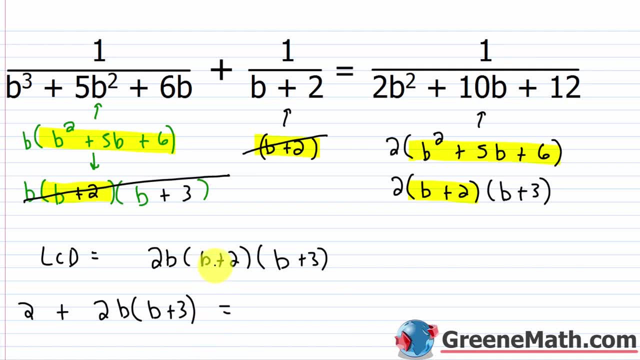 Then this equals: if I multiply 2b times the quantity b plus 2 times the quantity b plus 3 times this guy over here, what's going to happen is this will cancel. What will be left is just the b, So b times 1, which is just b. All right, so let's scroll down, get a little room going. 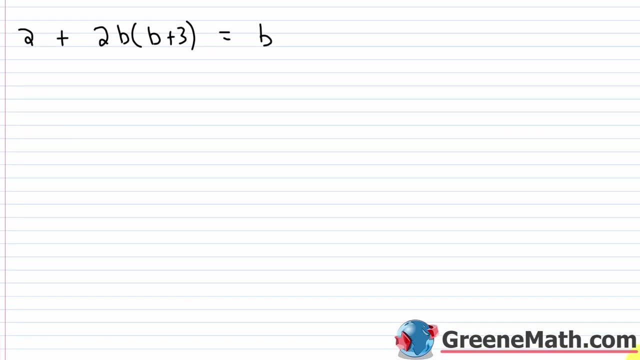 and we can solve this guy. So we can have: 2 plus 2b times b is 2b squared. then 2b times 3 is 6b and this equals b. So let's subtract b away from each side of the equation. 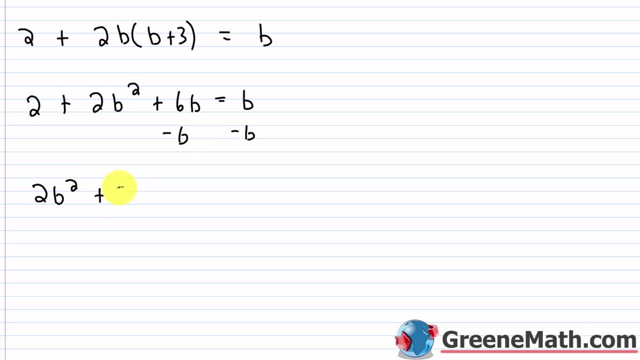 We'll have 2b squared plus 5b. then plus 2 is equal to 0.. Now I can't factor a 2 out because I have this 5 here. So what I'm going to do is I'm going to factor this using reverse FOIL. 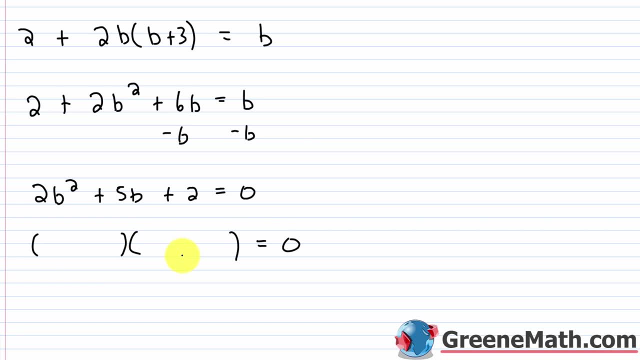 and I'm going to set each factor equal to 0, use my 0 product property and we'll get our solutions. So I know, if it's 2b squared, one of these would be 2b, the other would be b, and I just got to work out the outer and inner products now. 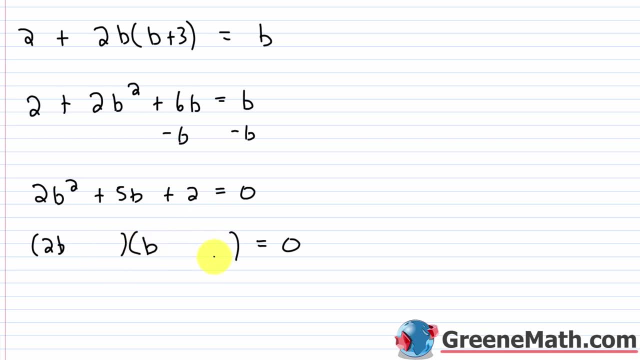 So I know that I want the last 2 to multiply together to be 2.. So really I know that's only 1 and 2.. I can't put a 2 here, because why? Well, the reason for that is there's no common factor. 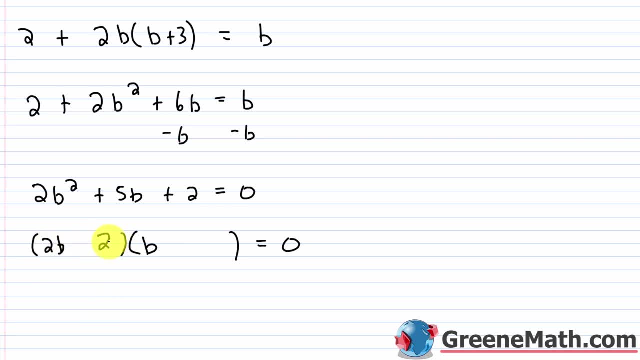 here. so there shouldn't be one in the binomial. This would produce a common factor 2.. So I've got to rearrange that and say plus 1 and plus 2.. Now does that work? Well, the outer would be what 4b, The inner would be what 1b. 4b plus 1b is 5b, Then 1 times 2 is 2.. 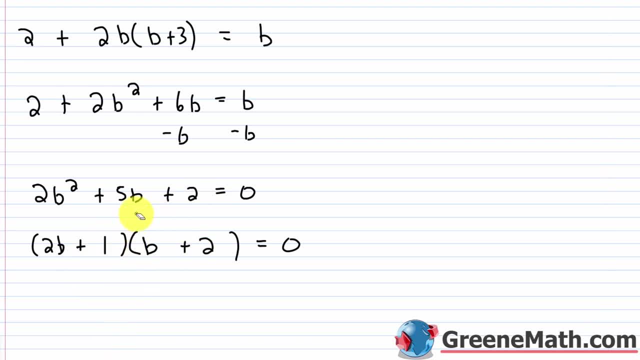 So we've correctly factored this guy. So now all we need to do is say 2b plus 1 is equal to 0, or b plus 2 is equal to 0.. Now let's see where that leads us. 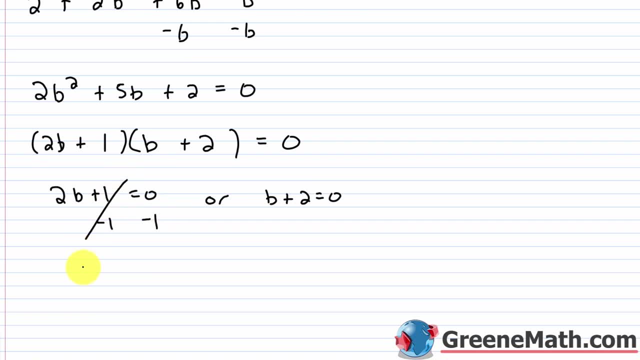 If I subtract 1 away from each side of the equation, I can't factor a 2 out, because I have 2b. If I subtract 2 away from each side of the equation, I'll have 2b is equal to negative 1.. 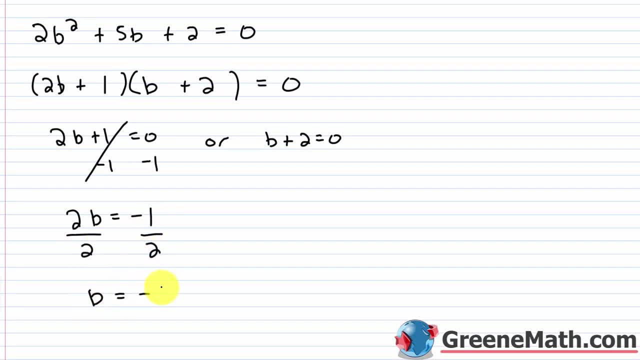 Divide both sides by 2. You'll have: b is equal to negative 1. half Over here we have. or If I subtract 2 away from each side of the equation, we'll have b is equal to negative 2.. This isn't. 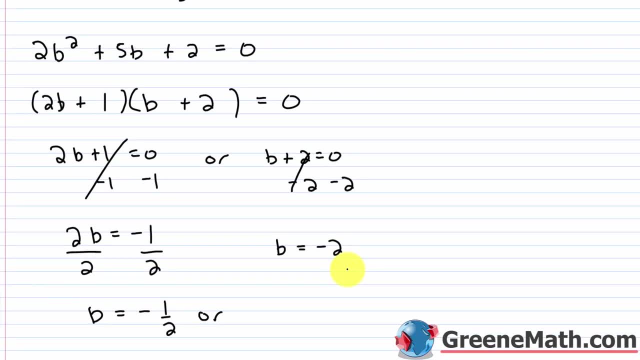 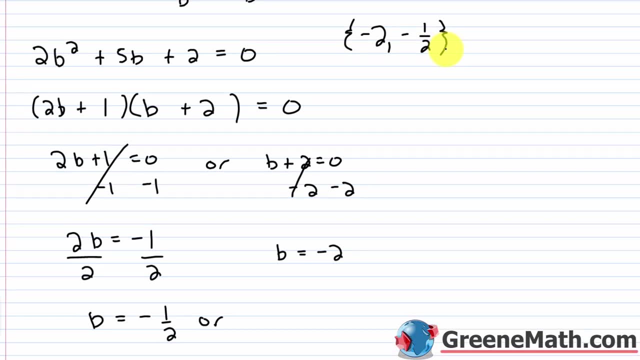 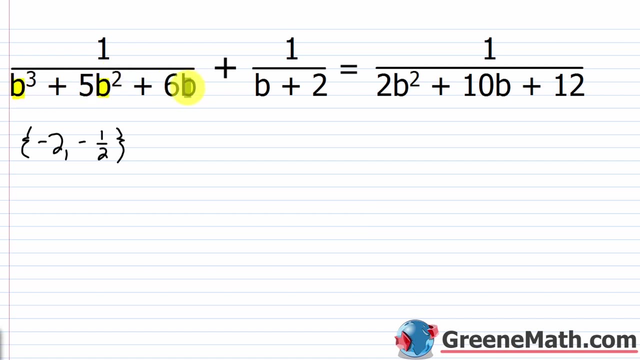 final, We've got to check these solutions to make sure they're valid. Right now let's just list it as negative 2 comma, negative 1 half, and then we'll check and make sure that those are valid. To check negative 2, I'm going to plug a negative 2 in: everywhere there's a b, So here here, here: 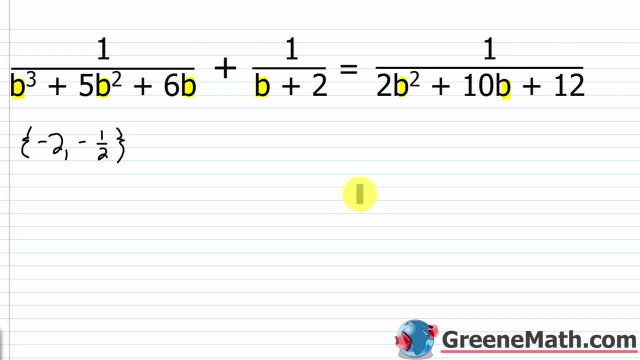 here, here and here. But before we even go through all that work, I want you to specifically notice this right here: If I plug in a negative 2 there, we're going to get negative 2 plus 2.. Negative 2 plus 2 is 0. So this right here would be 1 over 0. You cannot have that So. 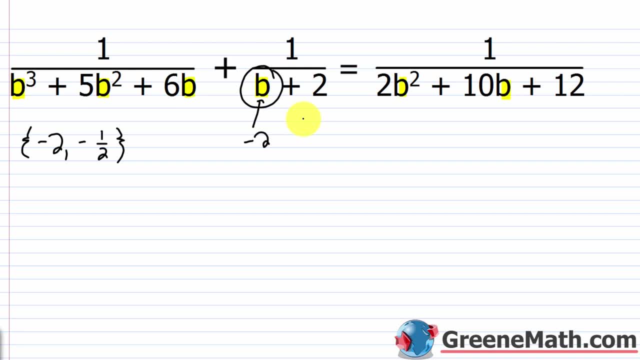 if you notice something like that, just stop. You have to reject that solution. So that is not valid. You have to reject it. So what we would try now is negative 1 half. So we would have 1 over. You'd have negative 1 half. 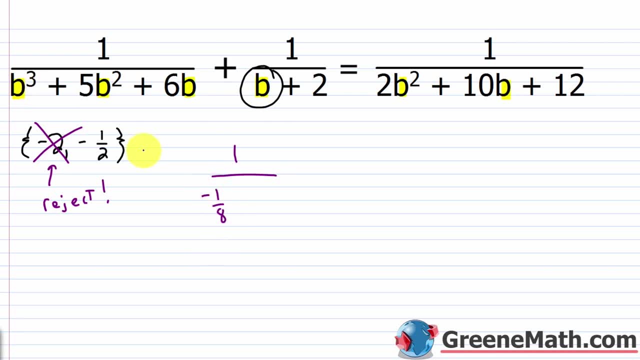 cubed. So that would be negative 1 eighth. Then plus You'd have negative 1 half squared, which would be positive 1 fourth times 5.. So it'd be 5 fourths. Then you'd have 6 times negative 1. 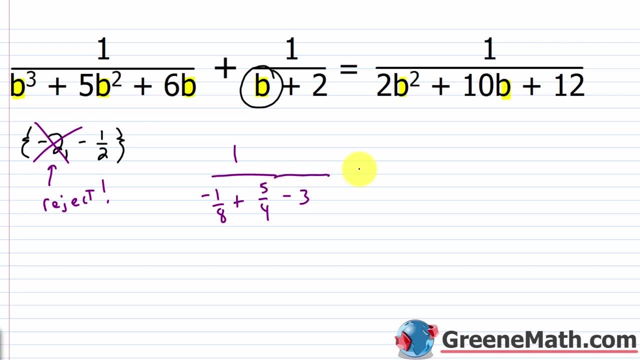 half, which would be negative 1 third. So you'd have negative 1 half cubed. So that would be so then you'd have plus. you have one over. you have negative one half plus two. so negative one half plus two. we'll simplify all this stuff in a minute. let me just drag this down here so we 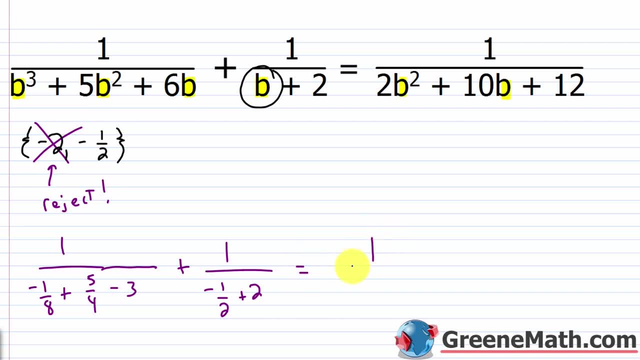 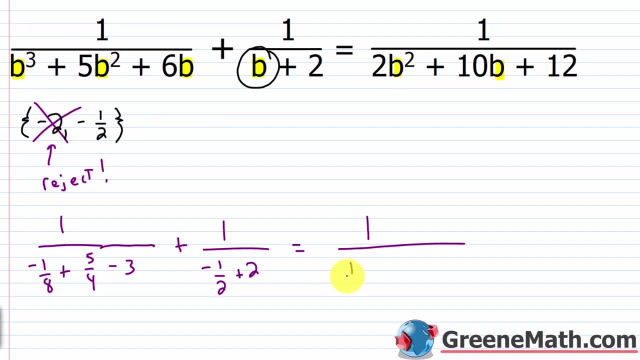 have some room, and then this equals: we have one over. if you squared negative one half, you'd have a fourth. a fourth times two would be a half. then plus 10 times negative one half is negative five. so you put minus five, if you want, and then plus 12, all right. so let's simplify this. see what we. 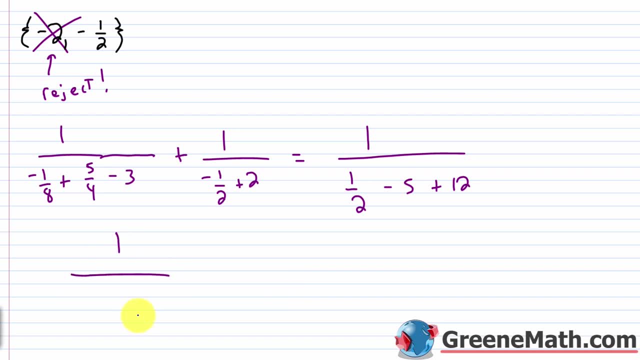 get, so we'd have one over. you have negative one. eighth plus five, fourths minus three. so to get a common denominator there, let's just go ahead and multiply this by two over two and multiply this by eight over eight, so you would have negative one plus 10 minus 24 over a common denominator. 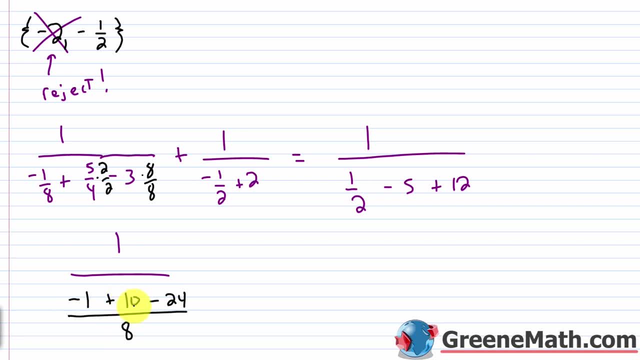 of eight, so negative one plus 10 is nine. nine minus 24 is negative 15. so if this is negative 15, here you've got to think about this as a division problem. it's basically one divided by negative 15 over eight. that's the same thing as if i said i had one times flip this guy. 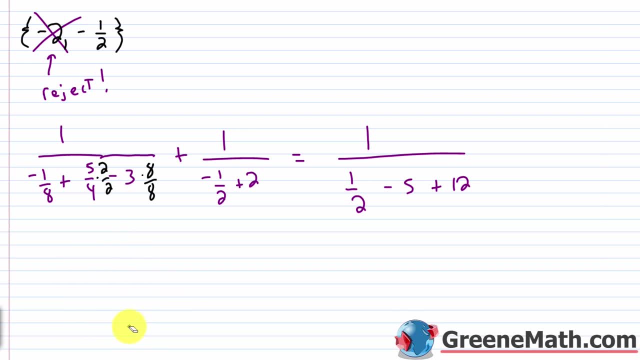 eight over negative 15. so this would be eight over negative 15 or negative eight. fifteenths. then you have plus here in the denominator. i would get a common denominator by multiplying by two over two. so you basically have negative one plus four, which is three over two. so this would be one. 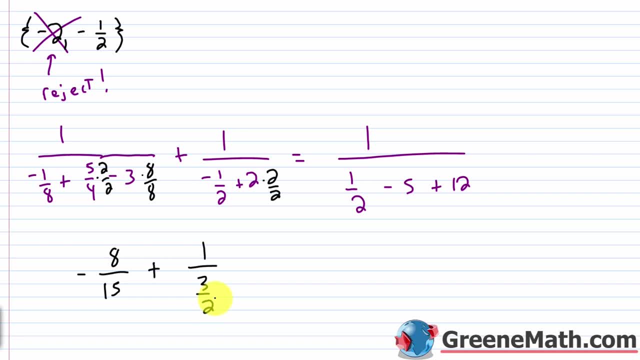 over three halves, which again is like one multiplied by the reciprocal of this. so this is two-thirds here. now to get a common denominator here, let's multiply this by five over five. two times five is ten. so this is ten, fifteenths now. ten plus negative eight is two. 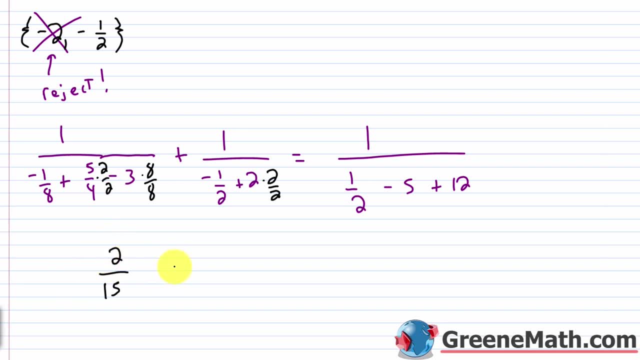 so the left side is just two fifteenths. this should be equal to this over here. so let's see what we get. so you get one half minus five plus twelve. so let's multiply this by two over two. let's multiply this by two over two, so we're going to have one over one minus ten plus twenty-four. 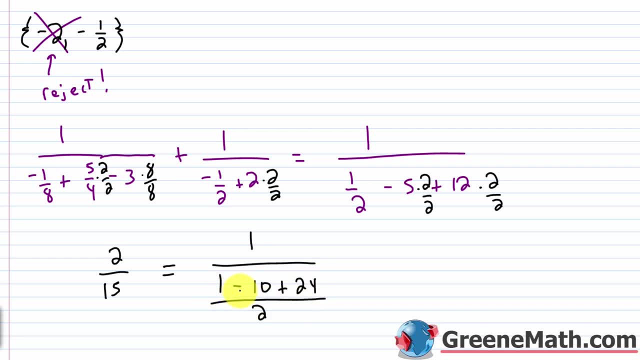 all over two. one minus ten is negative. nine negative. nine plus twenty-four is positive fifteen. this would be positive fifteen, so we're going to have one over one minus ten plus twenty-four positive fifteen. here and again i have one divided by fifteen halves, so it's like one times the. 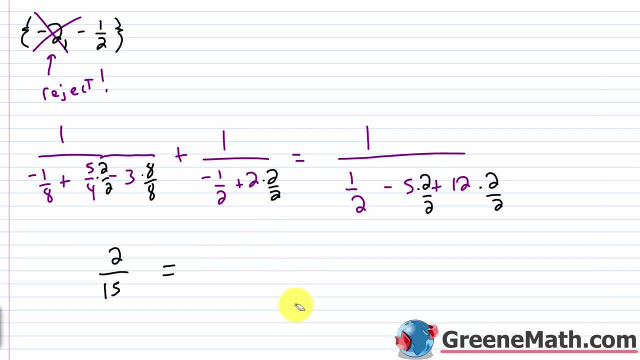 reciprocal of this one times two fifteenths, which is two fifteenths. so you get two fifteenths equals two fifteenths. so you know this solution is valid. let's put a check mark there. so really you can only say that b is equal to negative one half only. your solution set would just contain one element. 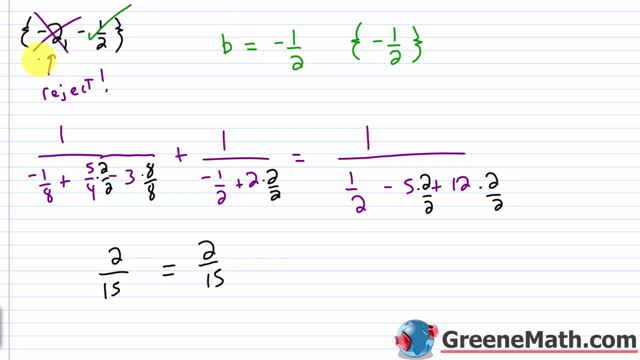 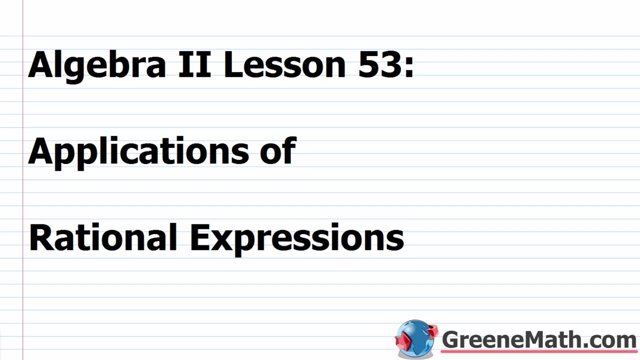 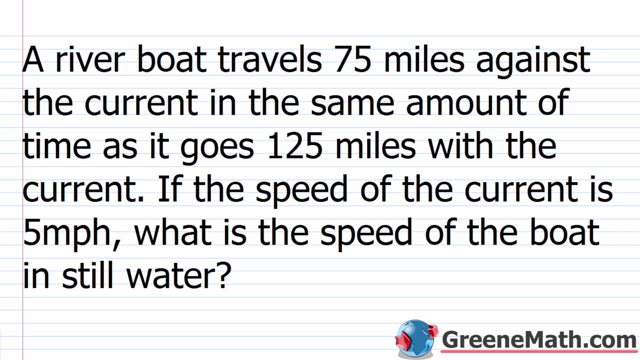 negative one half again. this negative two here that we found through solving the equation is not a valid solution. hello and welcome to algebra two, lesson fifty three. in this video we're going to learn about applications of rational expressions. all right, so at this point we should be very comfortable with solving word problems. all we're going to do in this lesson is: 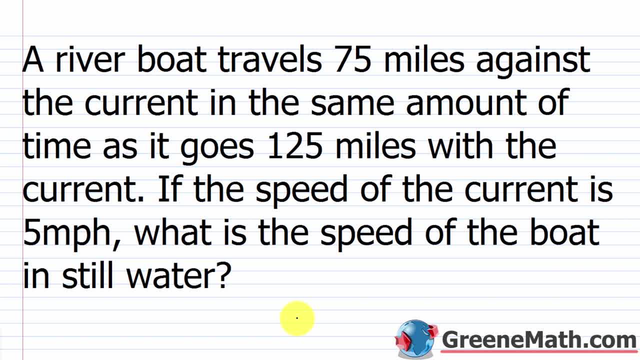 look at some examples where we deal with word problems, where we have to set up equations that have rational expressions involved. so not any more difficult than what we've been doing in the past, just a slight variation, and i just want to note that we did cover this in algebra one. it's just something we recover in. 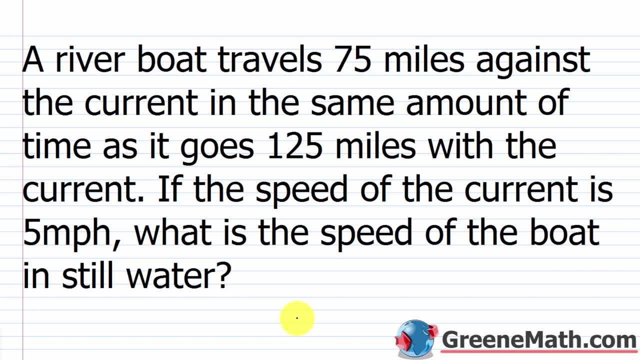 algebra two. so we make sure we fully understand something like this before we get into something more challenging. so i want to start out with this problem here. so we say that a riverboat travels 75 miles against the current and the same amount of time as it goes 125 miles with the current. 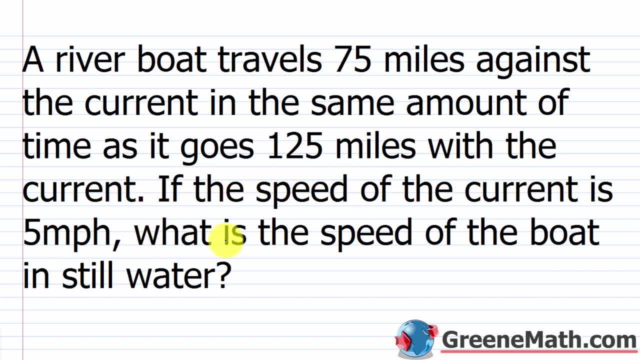 if the speed of the current is five miles per hour, what is the speed of the boat in still water? so what are we trying to find? we're trying to find out this right here: what is the speed of the boat in still water? so meaning, if there was no current? 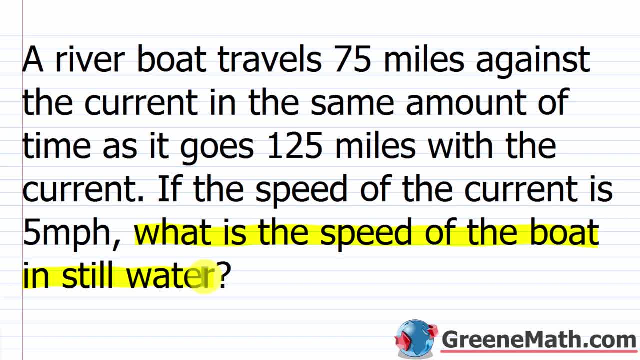 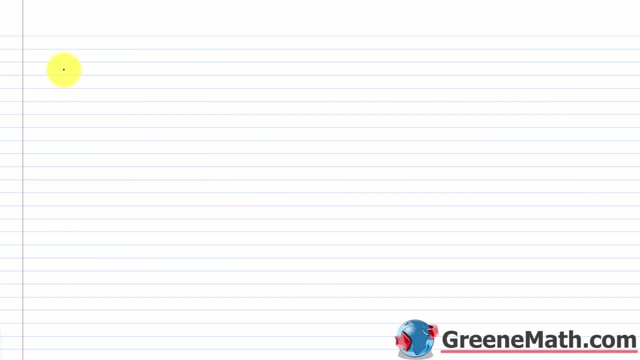 at all. well, to do this, we need to think about our distance formula. let's scroll down and think about the distance formula for a second. distance is equal to the rate of speed multiplied by the amount of time traveled. we all know if we're in a car, and i use this example all the time. 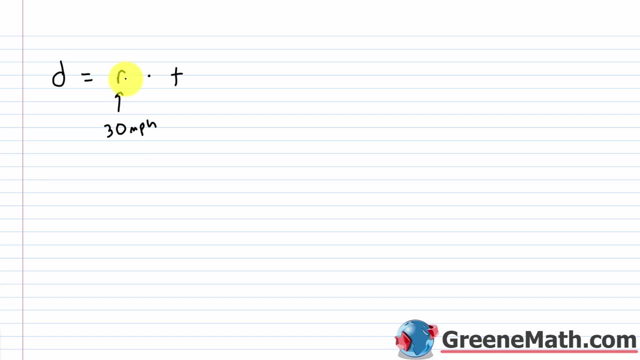 and we're driving, let's say, 30 miles per hour. that's our rate of speed, and we do this for, let's say, four hours. what's the distance going to be? we could work that in your head. just do 30 times four, that's 120.. this would be 120 and then for the units it would be miles, because we're dealing. 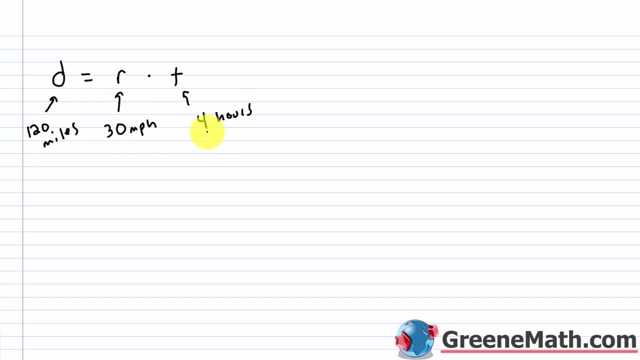 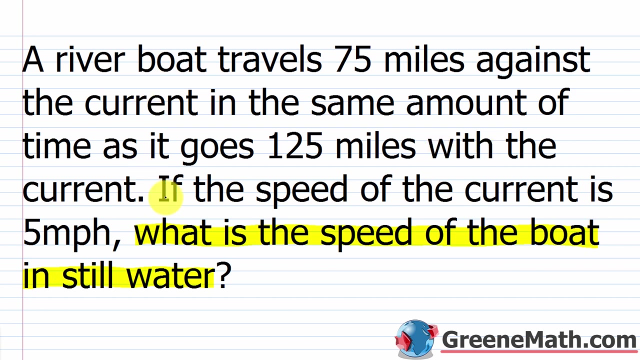 with miles per hour and hours. so we would go 120 miles in the future and we're going to do that in that scenario. now let's think about this formula with a nice little table. if we reread through the problem, we have two scenarios: we have against the current and we have with the current. so we have 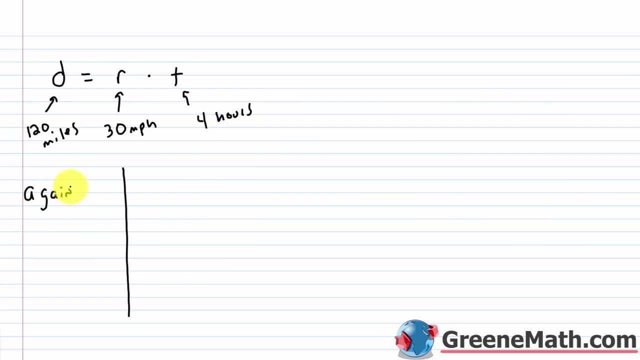 against the current, which i'll just label as against, and we have with the current, which i'll just label as width. so let's put: distance is equal to rate times, time like that, and we'll make ourselves a nice little table. i went over just a little bit, so let's kind of clean that up. 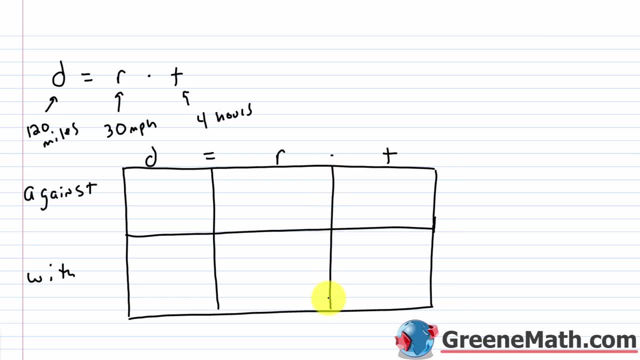 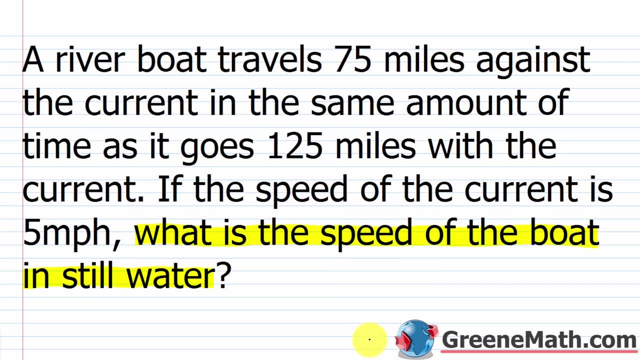 okay, let's make a little line here and now we're ready to go. all right, so the distance when we're going against and the distance when we're going with, let's see if we can fill that out. so it says that the riverboat travels 75 miles against the current, in the same amount of time as it goes: 100. 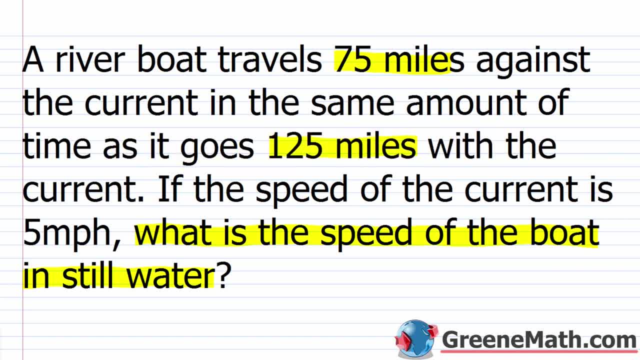 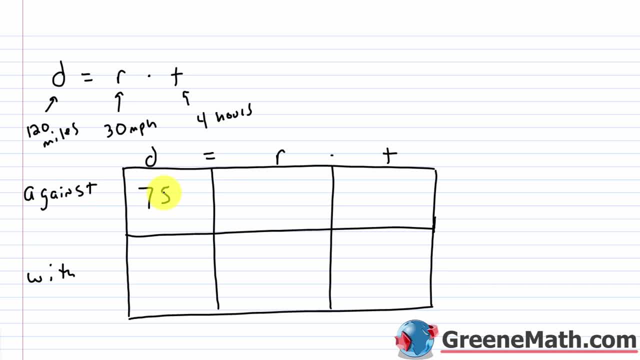 125 miles with the current. So when I'm filling this out the distance for against is going to be 75, right Short for 75 miles And then with width it's going to be 125.. Again, it's short. 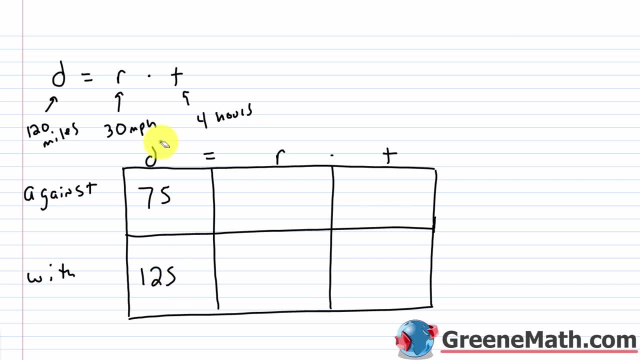 for 125 miles, And if you wanted to, you could go up here and just say, kind of, slide this over a little bit. This is in miles. Okay, now let's think about the rate of speed and the time. So for the 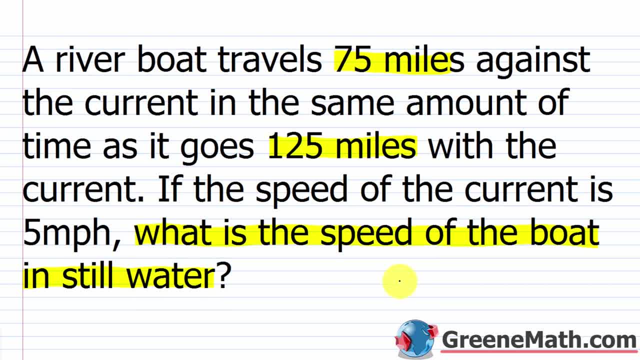 rate of speed. we're going to need to introduce a variable. All it tells us here is that the riverboat travels 75 miles against the current and the same amount of time as it goes 125 miles with the current. Now it says that the speed of the current is five miles per hour, but that's not a rate of. 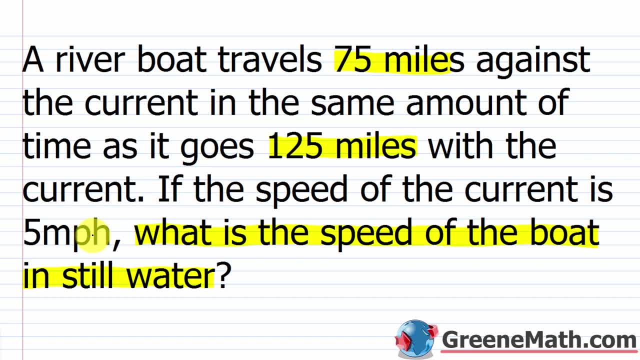 speed for the current. So we're going to need to introduce a variable, So we're going to need to the boat and how fast it's traveling. That's just a rate of speed for the current. The main question here is: what is the speed of the boat in still water? So let's go ahead and say that. 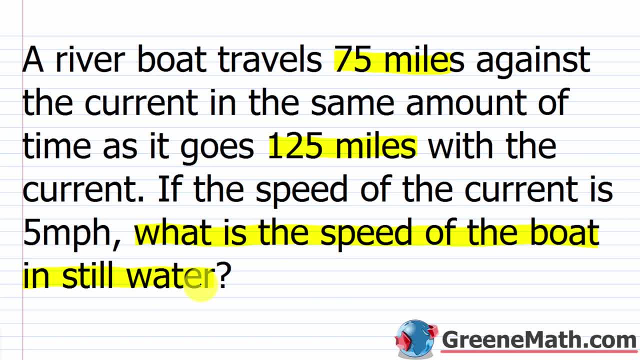 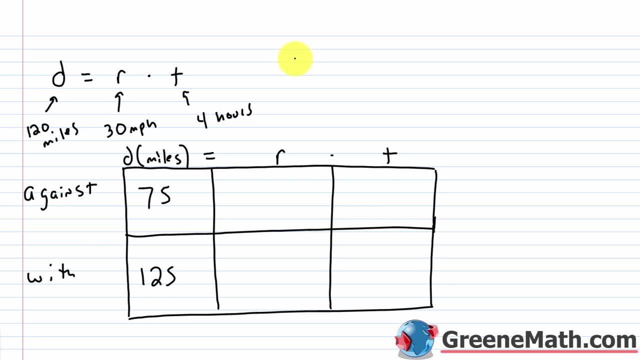 the unknown is how fast the boat is going to travel if there's no current involved, And then we can take this information here, this five miles per hour, the speed of the current, and we can add or subtract based on the scenario we're in. So if we say that we're going to let a variable 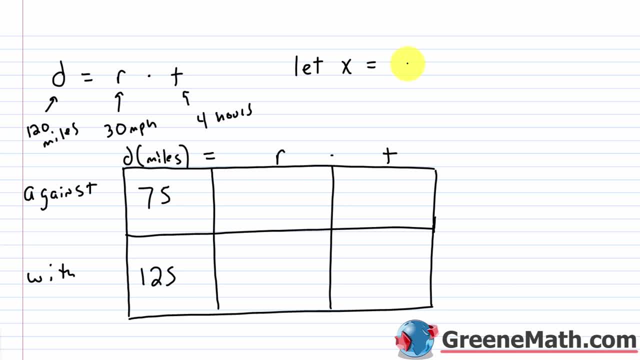 like x, be equal to the speed of the boat in still water, then what happens? Well, if we're fighting the current- which, again the current- let me just kind of make this on a side note- the current is what It's: five miles per hour. So if the rate of speed in still water is x- and I'm 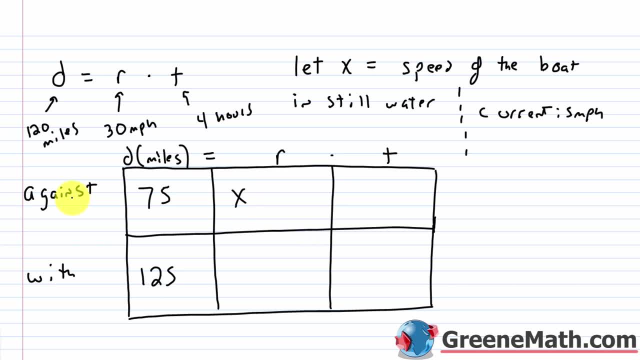 fighting the current, then I've got to subtract five away from whatever x is. Let's just say- and I'm not saying this is the answer- let's just say: the boat goes 30 miles per hour in still water. Well, if the current is five miles per hour and it's fighting us, well then we're going to take. 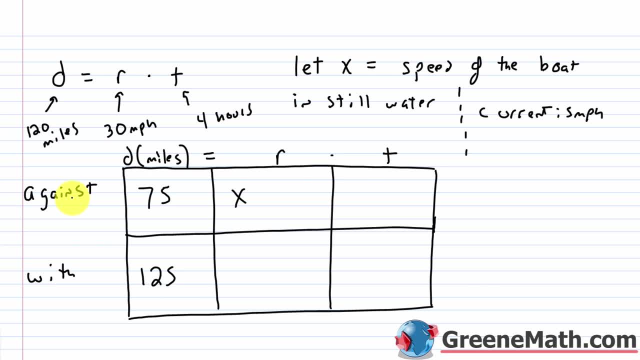 30 minus five and say we're going 25 miles per hour if we're going against the current. So I would subtract five away here. Now, when we go to with the current, now the current's pushing on the boat, It's making us fight the current. So if we're fighting the current then we're going to. 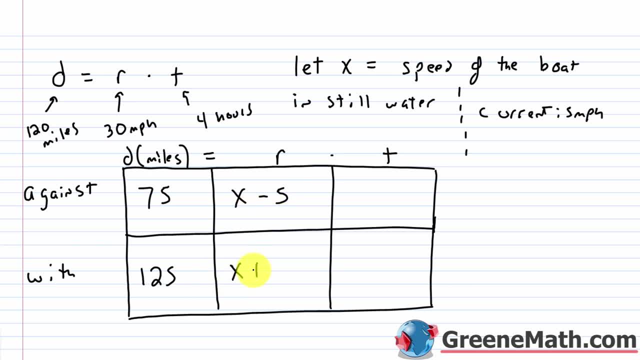 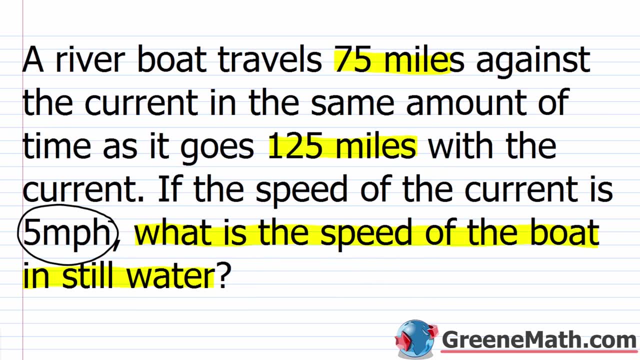 go faster. So I would add five, So I would have x plus five here. So now we have our rate done. So now let's think about time. So all it tells us, as far as information, is that the two times are equal. It says the same amount of time. Let me highlight that: Same amount of time, But it 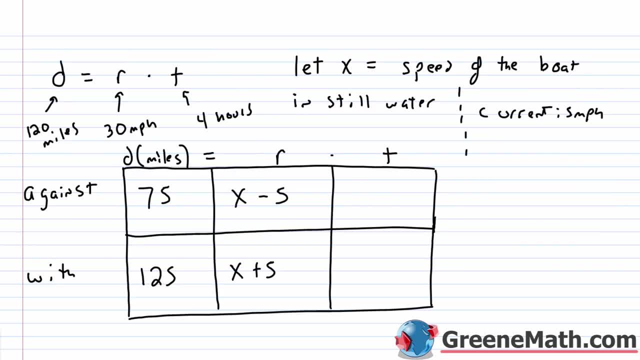 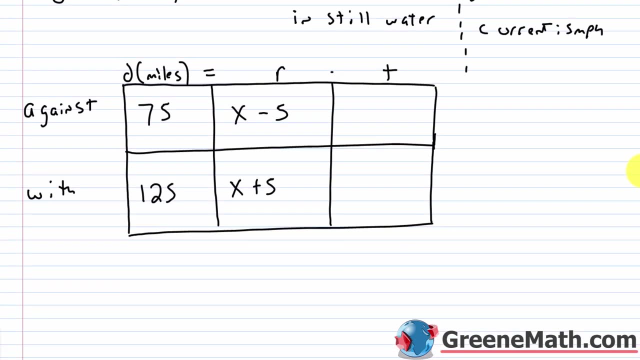 doesn't give us a time for either one, But fortunately with the distance formula, if you have two of them, you can get the third one right. They're doing a little bit of manipulation, So let's erase this for a second And let's just scroll down a little bit. If I wanted to solve for 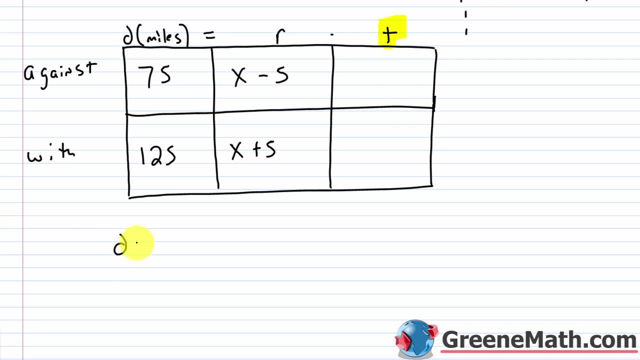 time, which is what I want to know, and I have. distance equals rate times time. I could divide both sides by r and I would have time on one side of the equation by itself. So time is equal to distance divided by rate. I have a distance here of 75. I have a rate of x minus five. So 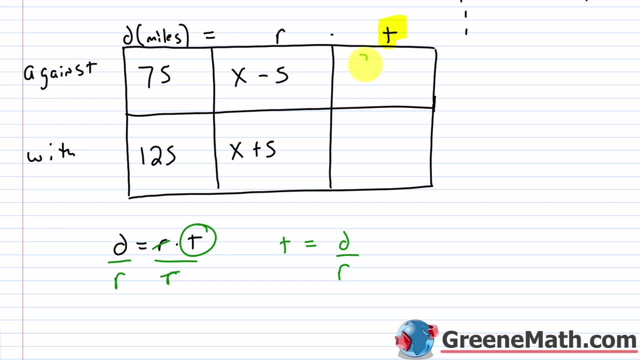 my time is equal to distance divided by rate. I have a rate of x minus five. So I have a rate of x minus five for this one, going against the current, is 75 divided by x minus 5.. For with the current, it's 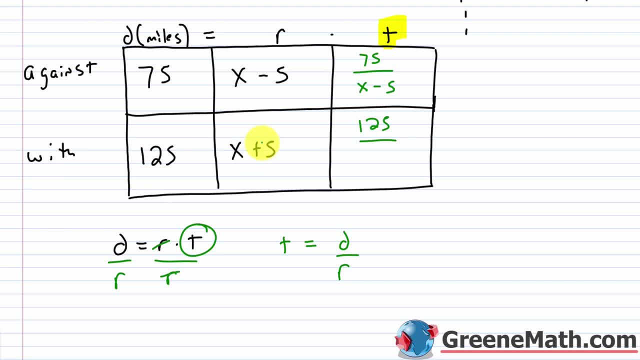 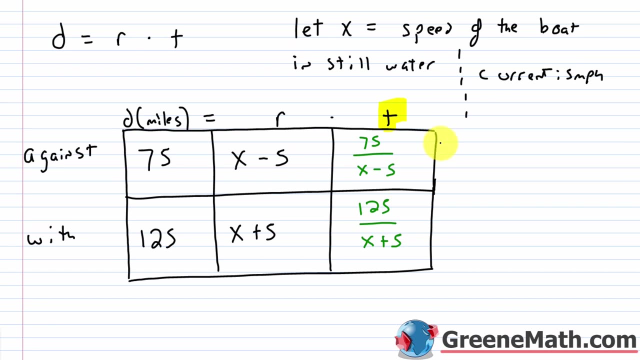 125, which is the distance divided by the rate of x plus 5.. So now we're beginning to see what we can do here. We've got our table filled out, so we have all the information we're going to need to gain a solution. The main thing here is that it says the two times are equal to each other, So the time 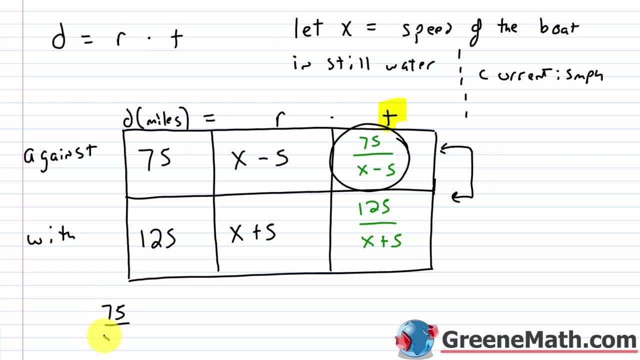 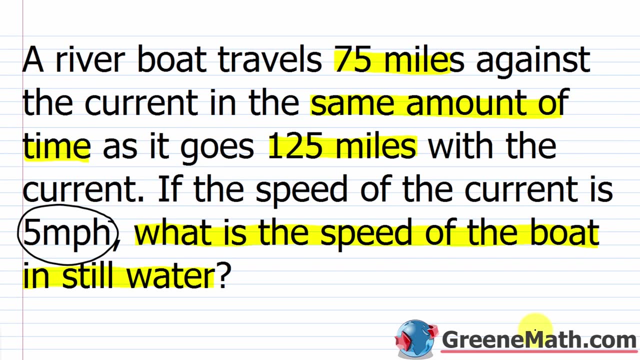 here, which is represented with 75 over x minus 5, is equal to, or the same as this time here, which is 125 over x plus 5.. Again, the way I'm getting this in the problem, it says in the same amount of time. 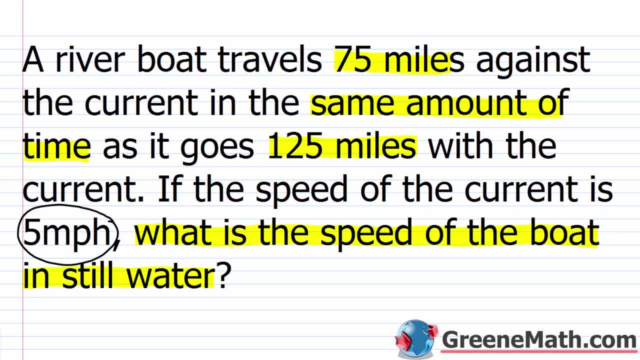 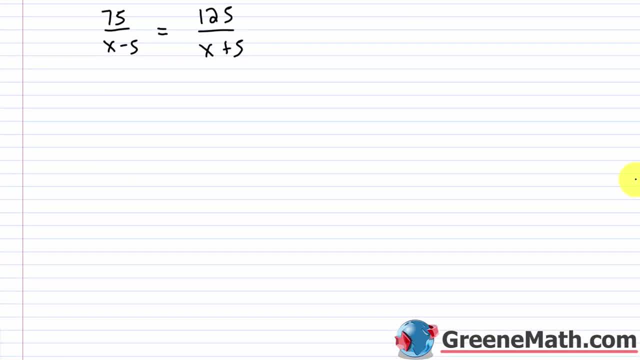 So again, the two times are equal. so that's how we get our equation. So now all we need to do is solve this equation for x, and remember x is representing the speed of the boat in still water. All right, so we can use the LCD method, or we can realize that we basically could just 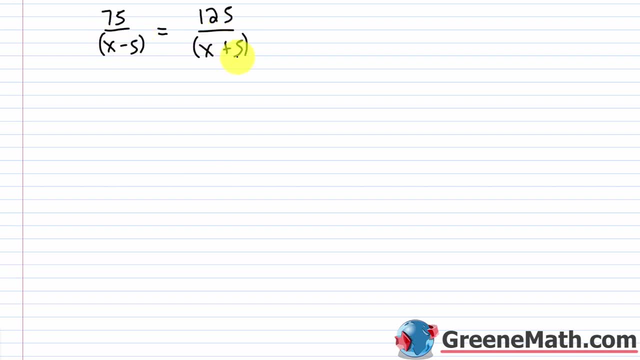 cross multiply here. Whatever you want to do, cross multiplying would be faster. Let's use our LCD method so we get some practice with that. The LCD would be what It would be: x minus 5 over x minus 5.. So that's the speed of the boat in still water. So we can use the LCD. 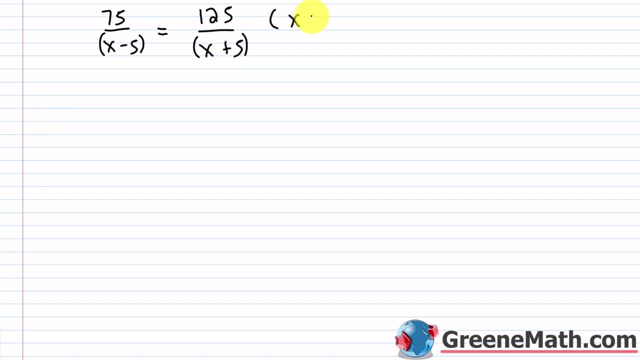 method, or we can realize that we basically could just cross multiply here Whatever you want to do. cross multiply here Whatever you want to do, cross multiplying here, Whatever you want to do. cross 5 over x minus 5 and we're gonna just lay down a little harder and do what that way. The x. 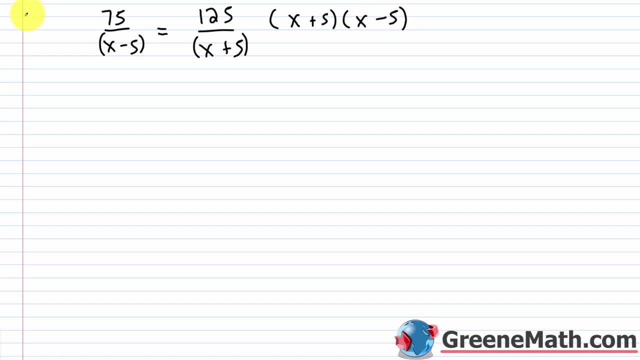 reinforced of x-5 times x-5, and the size of one page is equal to x minus 5 over x-5 minus 5.. So I multiply this by x plus 5 times x minus- funny Over here- by x plus 5 times x minus. 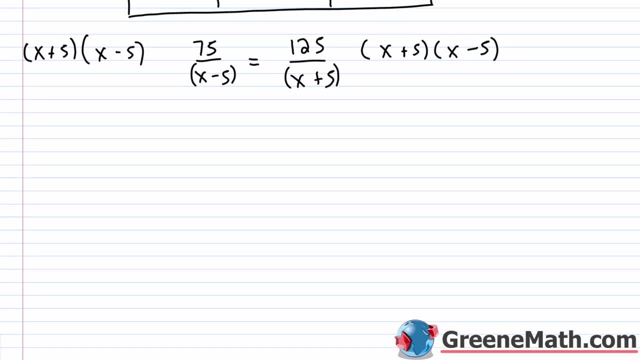 5 and over here by x plus 5 times x minus 5.. And what is this going to do for us? Well, in this case, this would cancel with this. over here, this would cancel with this, and so you're left with is equal to 125 times the quantity x minus 5.. 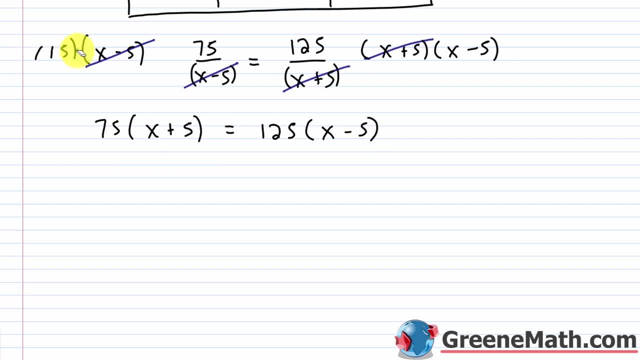 And again, you could have got the same thing by just cross-multiplying. If I erase this, what could I have done If I multiply this by this? that's what I've got here- And then it would be equal to this times. this, that's what I've got here. 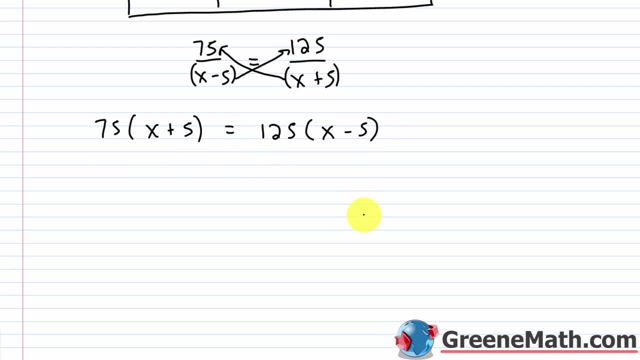 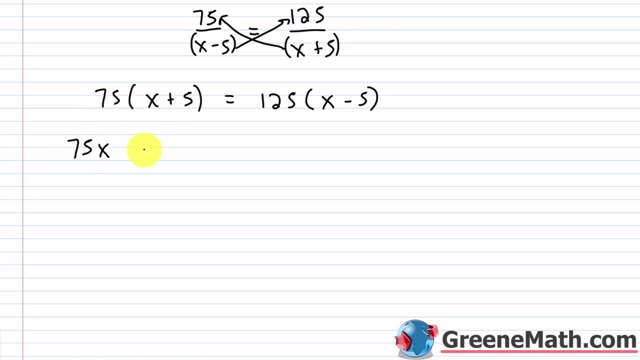 Right. so the easier thing to do in that scenario would have been to just cross-multiply, All right. so 75 times x is 75x, And then 75 times 5 is 375, so plus 375.. This equals 125 times x is 125x. 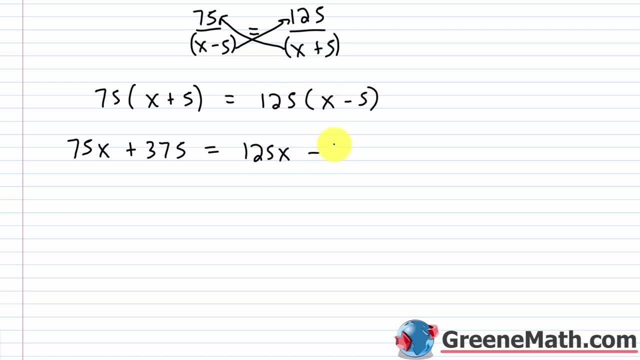 And then 125 times negative 5 is negative 625.. All right, so what we want to do here? let's subtract 125x away from each side of the equation So that'll cancel, And let's subtract 375 away from each side of the equation. 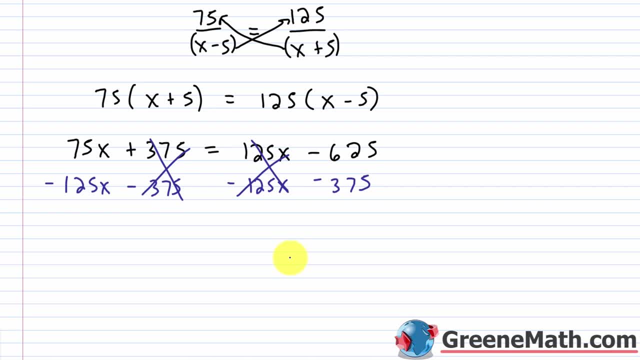 So that'll cancel. So 75x minus 125x is negative 50x. This will be equal to negative 625 minus 375 is negative 1,000.. So to finish this off, let's just divide both sides of the equation by negative 50.. 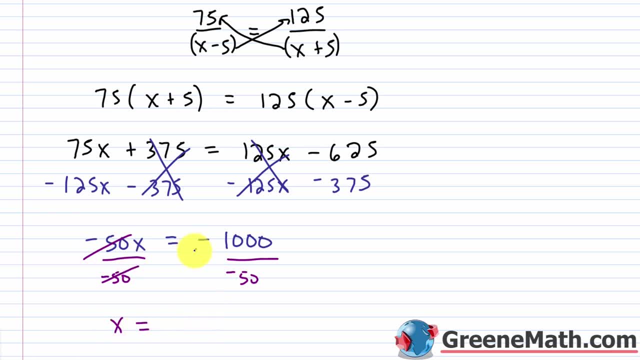 So this will cancel. You'll have: x is equal to negative over negative is positive, And you can cancel a zero here. You'd have 100 divided by 5, which is 20.. So x equals positive 20.. So again, when we have a word problem, we can't just stop and say x equals 20 and say, oh, we're done. 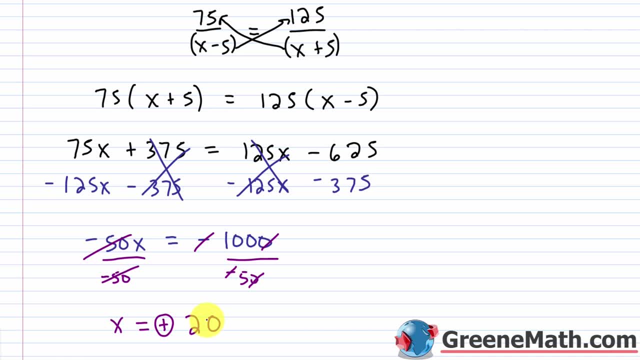 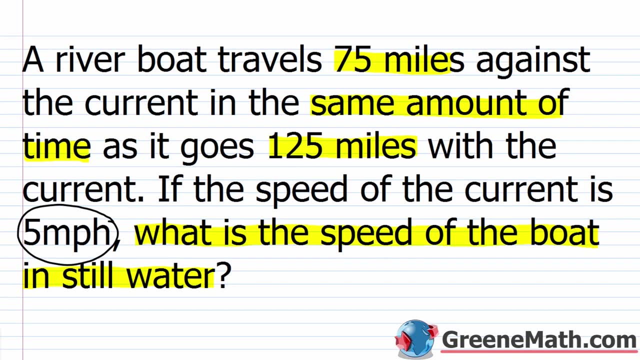 It doesn't work that way. We have to think about what this actually means. Remember, x was the speed of the boat in still water. That's what we're trying to find to answer the question: What is the speed of the boat in still water? 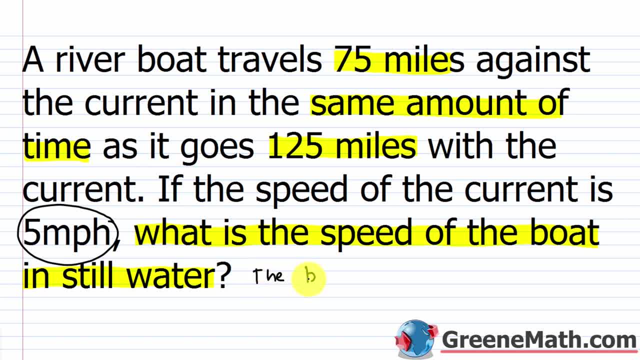 Well, the speed of the boat, Or we could say the boat travels at 20 miles per hour in still water. Now, does that make sense in terms of the problem? Well, a riverboat travels 75 miles against the current. So 75 miles against the current. 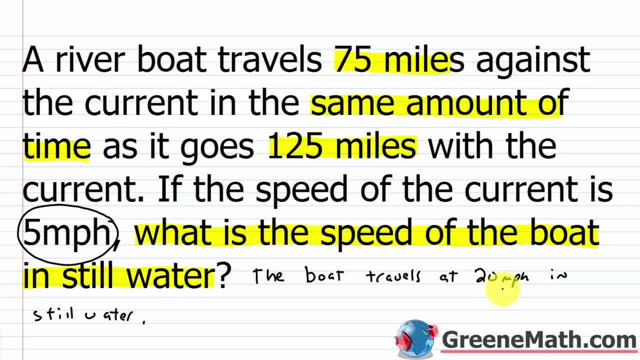 If the boat travels 20 miles per hour in still water, if it's fighting the current and the current's 5 miles per hour, that means it's going 15 miles per hour. So to go 75 miles at 15 miles per hour that would take 5 hours. 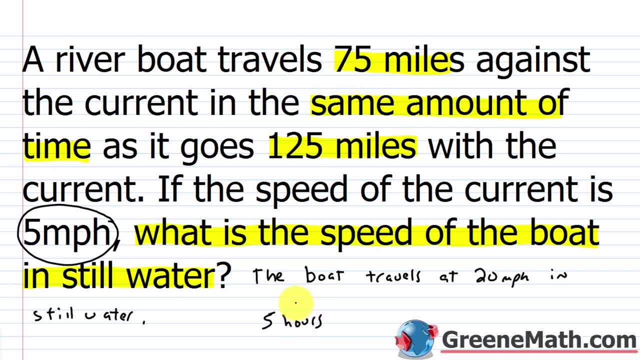 So it would take 5 hours. Now it says same amount of time as it goes: 125 miles with the current. So in 5 hours with the current, if I go with the current here, I'd take 20 miles per hour. 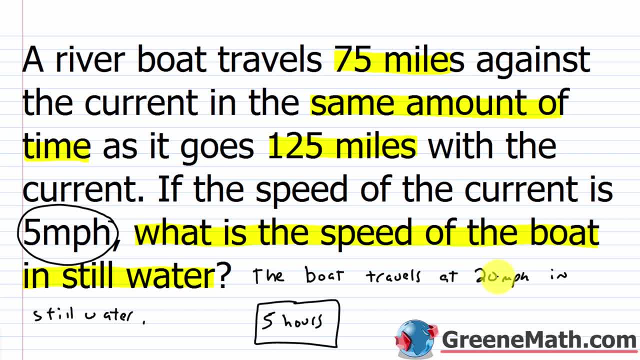 and I would add the speed of the current, So now it's 25 miles per hour. What would that do in 5 hours? Well, 25 times 5 is 125. So that's accurate. It would go 125 miles in the same amount of time as it goes 75 miles. 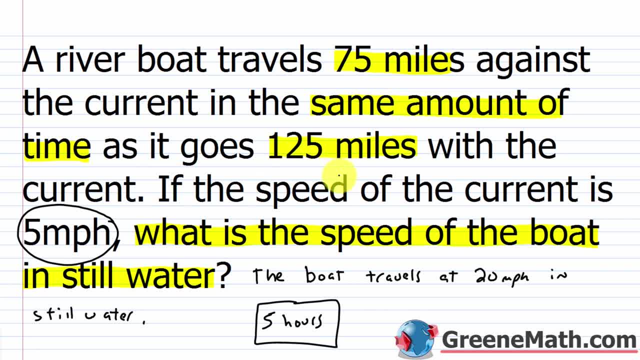 So the boat would in fact travel 125 miles with the current in the same amount of time, the 5 hours as it takes to go 75 miles traveling against the current. So we have the correct answer here Again: the boat travels. 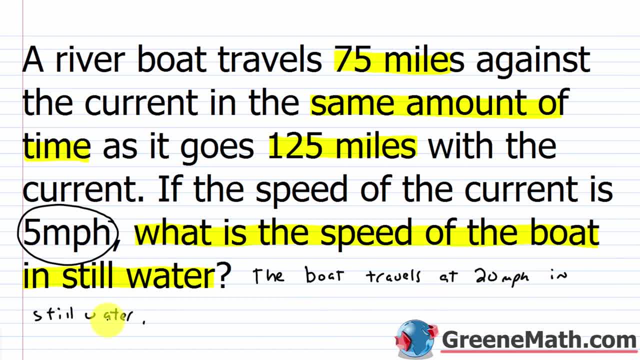 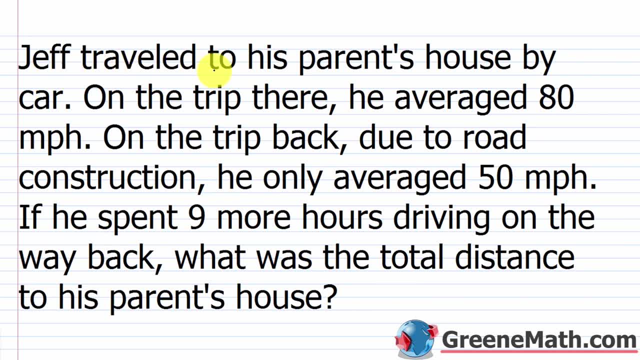 The boat travels at 20 miles per hour in still water. Well, let's take a look at another one that involves this distance formula or, again, a motion word problem. So Jeff traveled to his parents' house by car. On the trip there, he averaged 80 miles per hour. 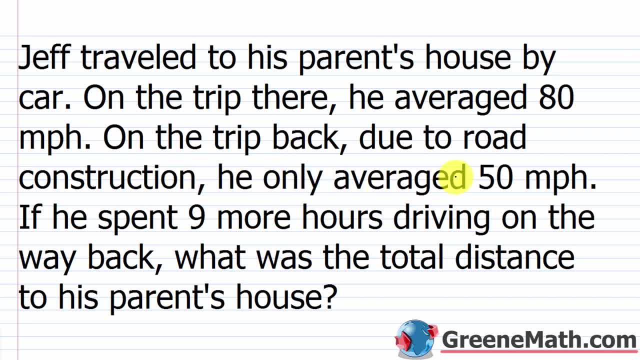 On the trip back, due to road construction, he only averaged 50 miles per hour. If he spent 9 more hours driving on the way back, what was the total distance to his parents' house? So you might look at this, You might look at this problem and just be really confused on how to get started. 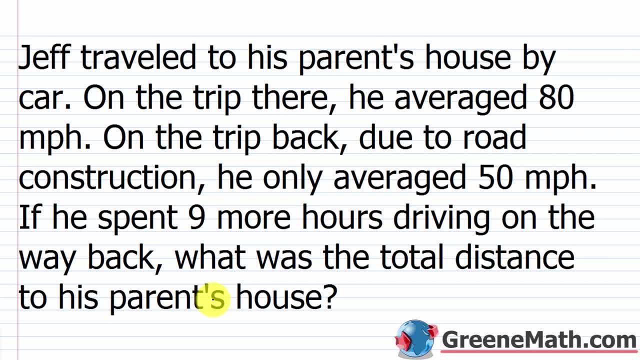 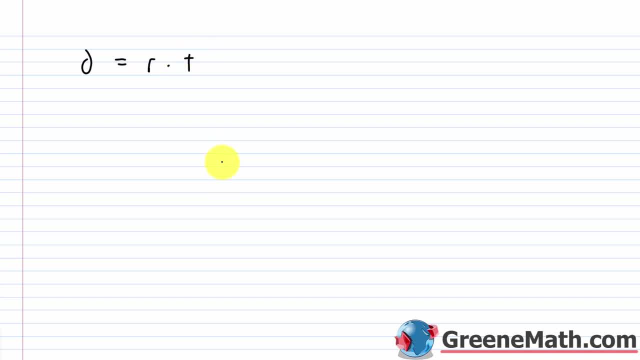 It doesn't seem as simple or as straightforward as the last problem. But again, if you go back to that distance formula, if you just say distance is equal to rate, times, time, and you make yourself a little table, okay, this is a great way to just organize your information. 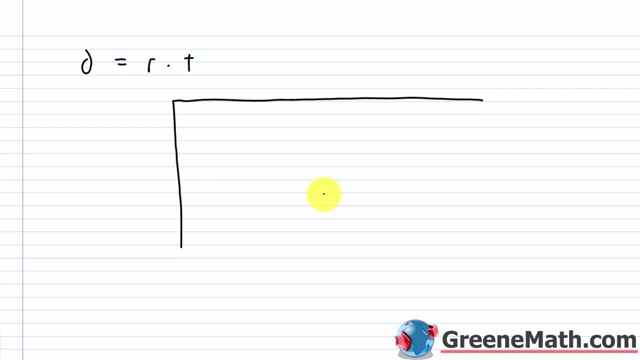 So we have a trip to his parents and a trip back from his parents. So there's the trip there And there's the trip back. So those are your two different scenarios. Okay, so let's write. distance here is equal to rate times time. 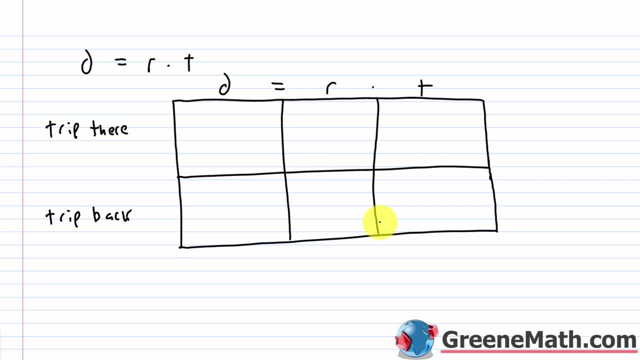 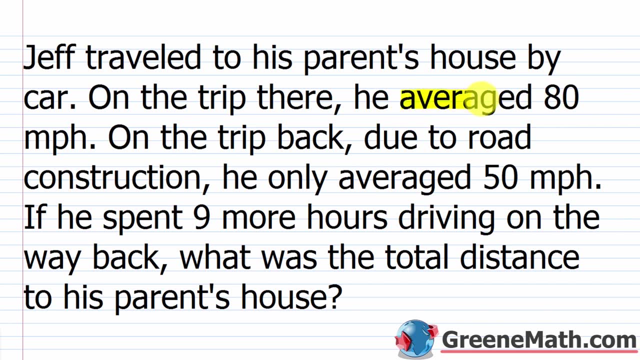 All right. so let's go back up and see what we can figure out. So the first information we're given is that on the trip there he averaged 80 miles per hour. So he averaged 80 miles per hour. So that is something we're going to write under rate. 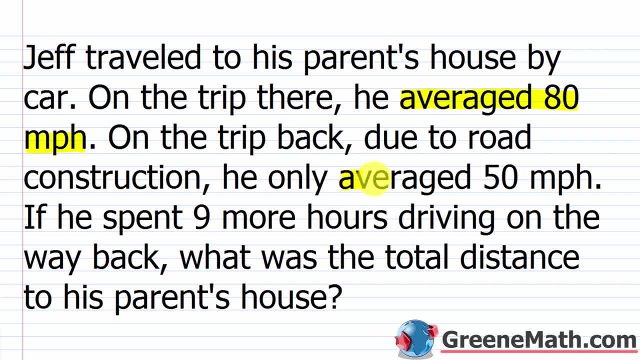 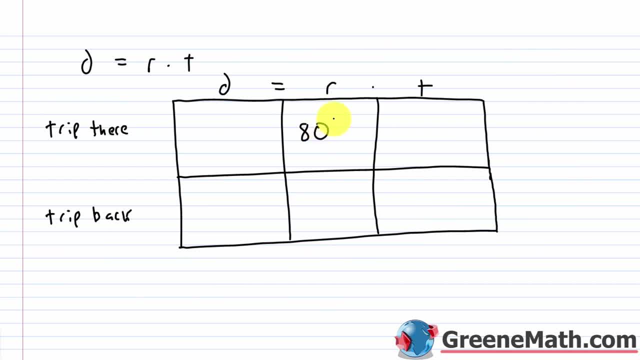 Now it says: on the trip back he averaged only 50 miles per hour. So let's put those in under rate. So for the trip there it was 80 miles per hour. On the trip back it was only 50.. 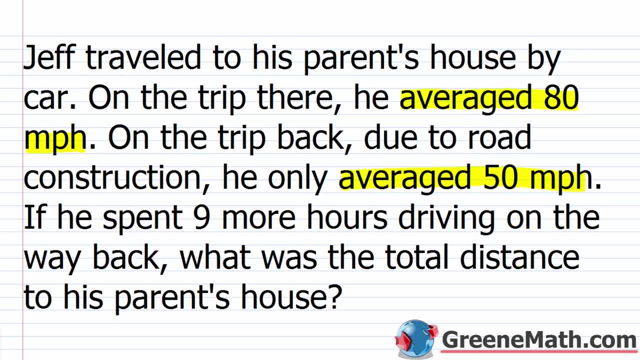 Now, when we start talking about distance, remember the main question here is: what was the total distance to his parents' house? What was the total distance? What was the total distance to his parents' house? So we don't know that. 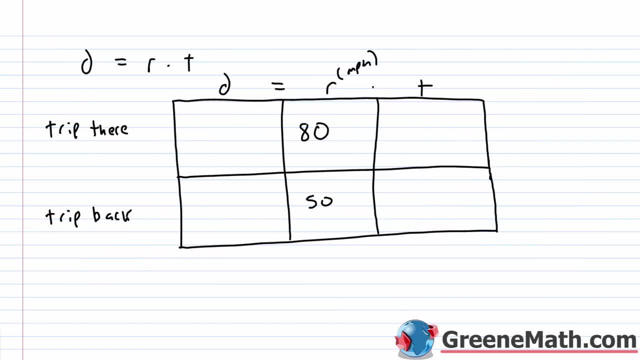 So if it's an unknown, let's assign a variable to represent it. So let's say that we're going to let x be equal to the distance- and this is in miles- to his parents' house. So we put x for the trip there and x for the trip back, because the distance is the same. 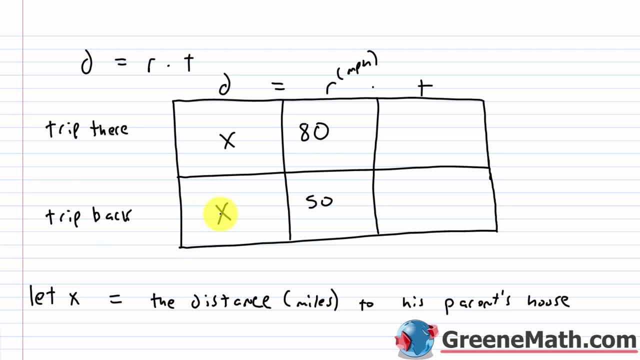 Now, what about time? Again, we saw this in the last section, where we said that we could find time by algebraically manipulating this formula. If I divide both sides of this equation by r, I would have that distance over rate is equal to time. 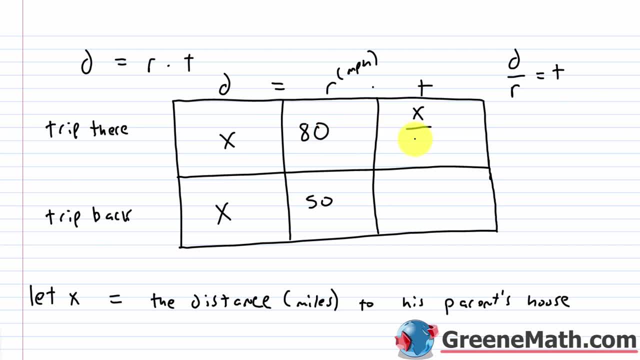 So I have a distance of x over a rate of 80, so that's my time for the trip there. For the trip back, I have a distance of x over a rate of 50, so x over 50 is my time for the trip back. 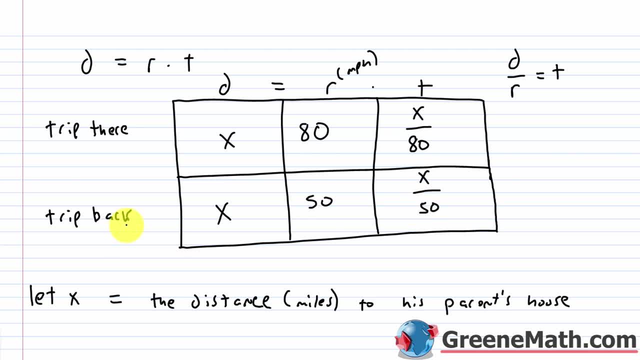 Now, how do we set up an equation? The times are not equal like they were in the last problem. We can't say this is equal to this. It's not that straightforward here. We have to read back through the problem and think about this. 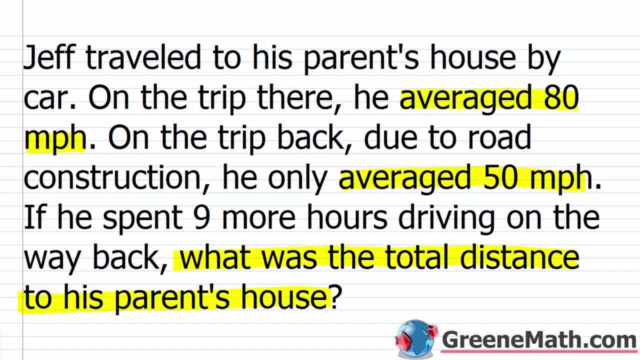 So Jeff traveled to his parents' house by car. On the trip there, he averaged 80 miles per hour. On the trip back, due to road construction, he only averaged 50 miles per hour. Now this is going to be the key to setting up an equation. 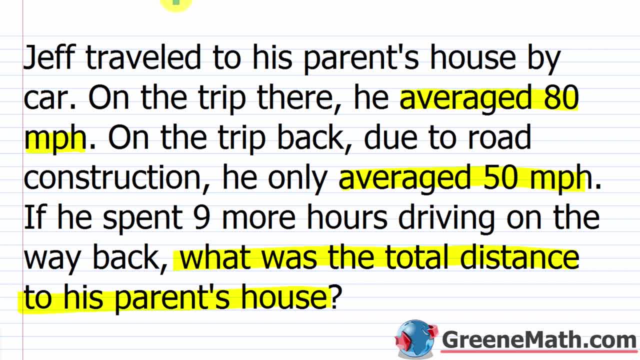 You always look for information that they give you that allows you to do this. If he spent nine more hours driving on the way back, just stop for a second. We know that the time driving on the way back was nine hours, more than whatever it was driving there. 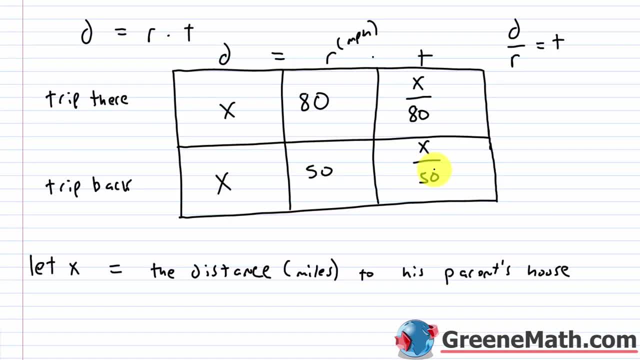 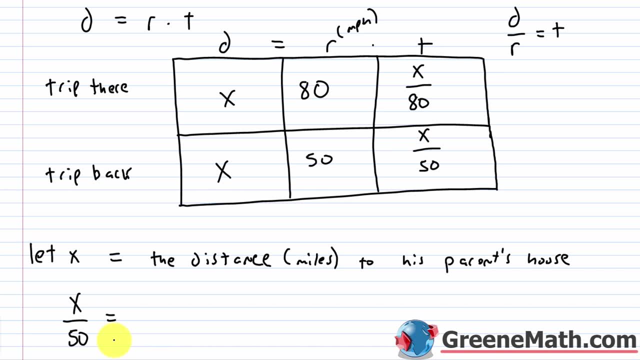 So we know that the trip back is going to take us nine hours more. So that means x over 50,, which is the time for the trip back would be equal to or the same as the time for the trip there, which is x over 80,. 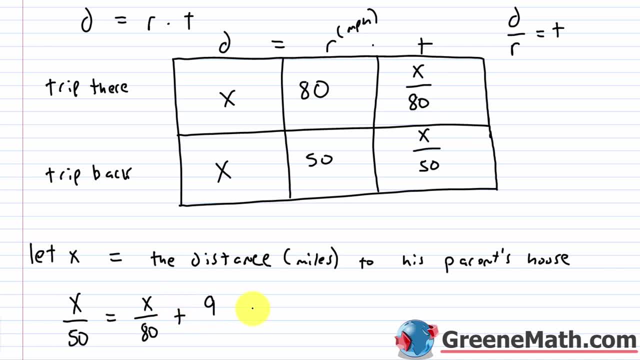 plus an additional nine hours. Right, Because again, the trip back is equal to or the same as the time for the trip there, which is x over 80, plus it takes another nine hours. So this would be the equation that you want to run with. 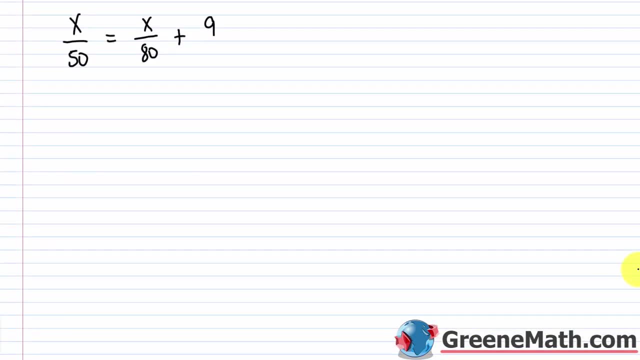 Now to solve this. I just want to find my LCD. So what's the LCD? If I look at the denominators here, I have 50 and I have 80. If I factored 50, I would get what. 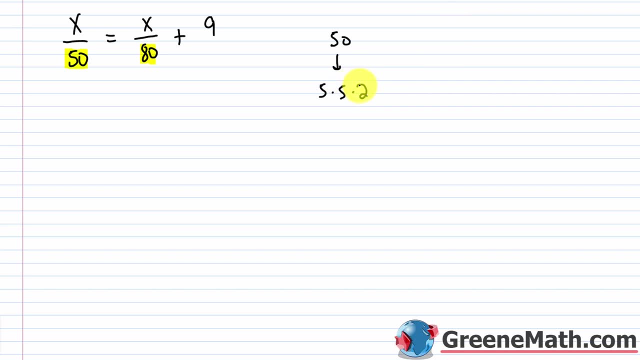 I would get 5 times 5 times 2.. Right, Basically 25 times 2.. If I factored 80,, 80 is what It's 16 times 5.. So 16 is 2 to the fourth power times. 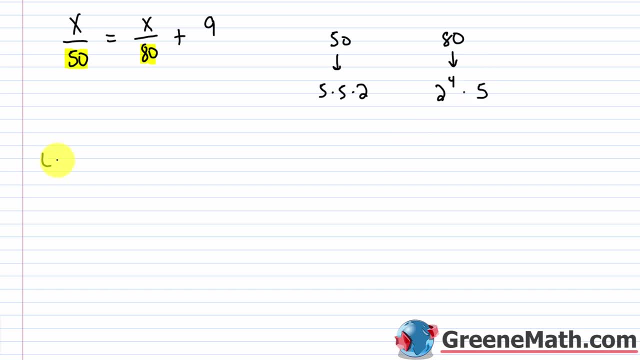 and then again you'd have 5.. So for my LCD I would have 2 factors of 5, or 25, multiplied by 4 factors of 2, or 16,, so this is 400.. So we basically take 400. 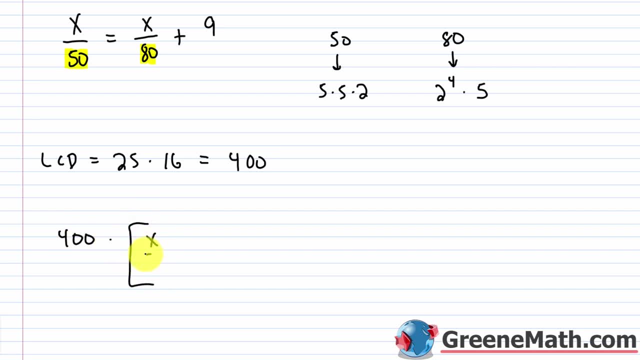 and multiply it by what You have x over 50,, and then this equals you'd have x over 80, plus 9, and you're multiplying this side by 400 as well. So this is going to clear all the denials. 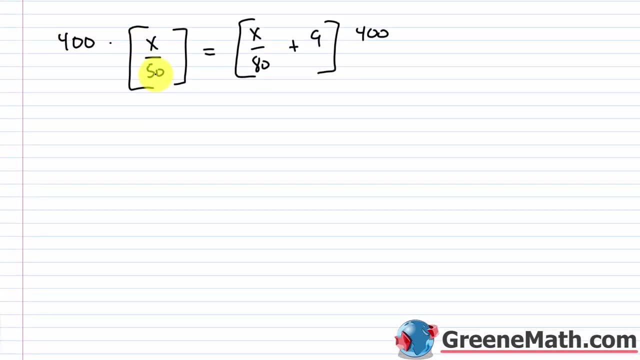 all the denominators for us. If I multiply 400 times x over 50,, the 400 would cancel with the 50, and give us an 8.. So this would be 8 times x, or just 8x, And this is equal to. 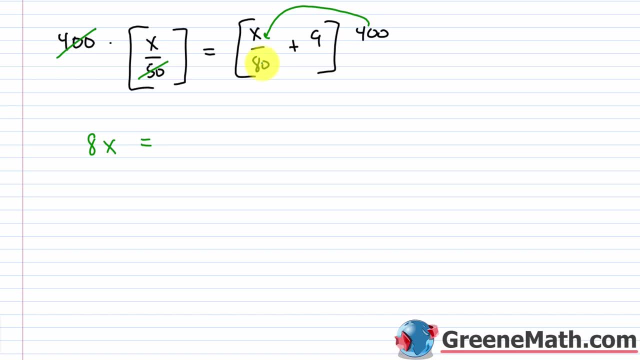 if I do 400 times x over 80, the 400 would cancel with the 80 and give us a 5, so you'd have 5 times x or 5x, And then plus if you did 400 times 9,. 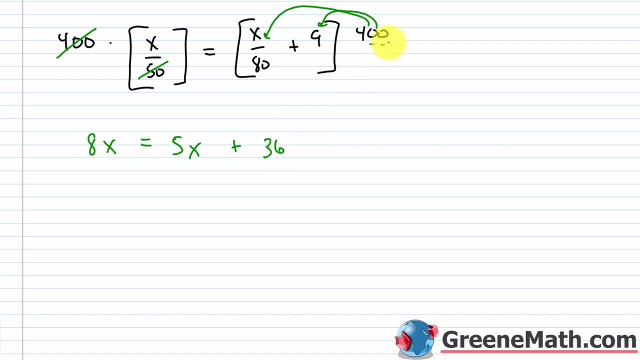 the quick way to do that: 4 times 9 is 36, and that goes at the end, so you'd have 3600 there. Alright, so to solve the equation, let's subtract 5x away from each side. 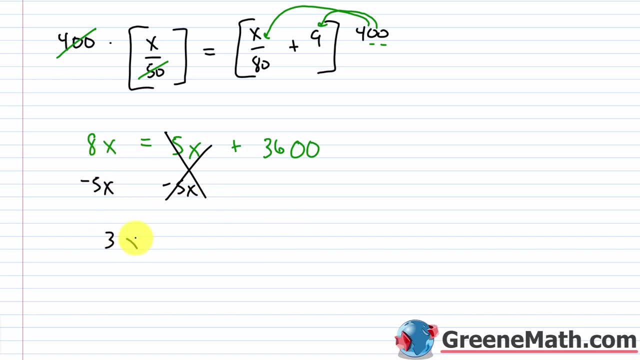 So this will cancel. 8x minus 5x is 3x, This is equal to 3600.. We'll now divide both sides of the equation by 3, and we get that x is equal to 1200.. Alright, so let's go back up to the top. 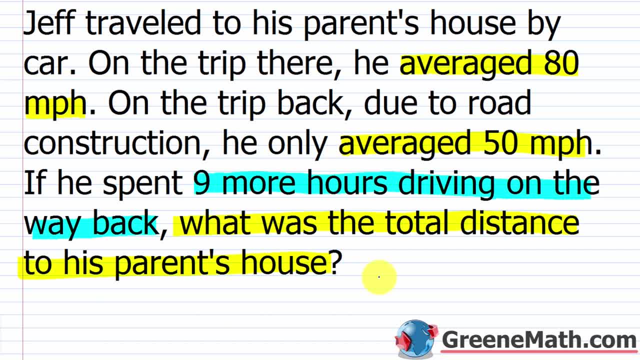 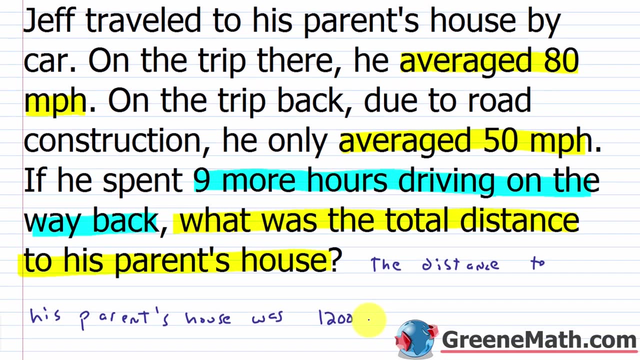 We said that the distance to his parents' house, or the total distance to his parents' house, was represented with x. we just found out that x was 1200, so we'll say the distance to his parents' house was 1200 miles. 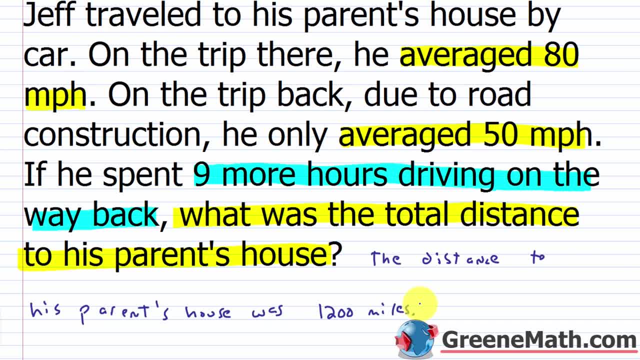 And it's pretty easy to check that Again if you can just move the distance formula around based on what you need. it's easy to check things like this. So, if you think about averaging 80 miles per hour and you're trying to go 1200 miles, 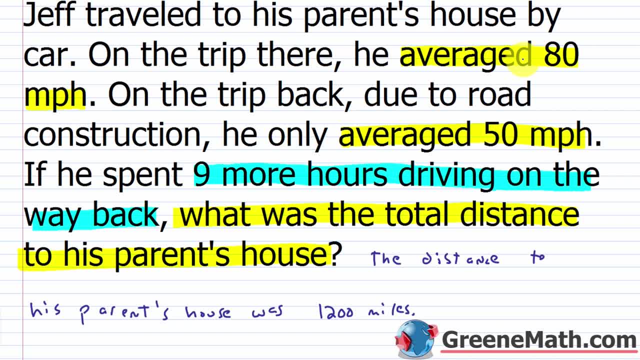 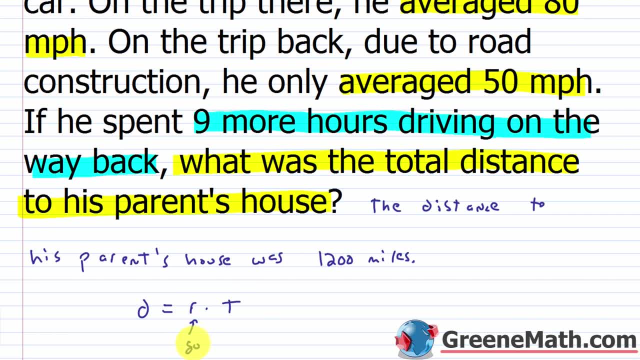 that's something you can calculate all the time, right, if you're doing a road trip. So I know that. again, distance equals rate times, time. So if the rate is 80, and the distance is 1200,, again to calculate the time, 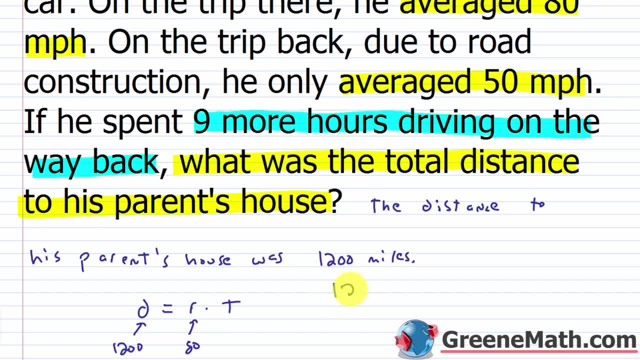 I would divide the distance by the rate. So what is 1200 divided by 80?? That's going to give me what? Well, it's going to give us 15.. So the amount of time for the trip there was 15 hours. 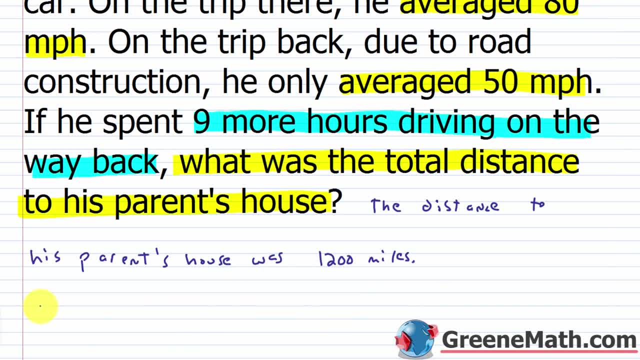 So for the trip there, let's just notate that for the trip there it was 15 hours. Now what about the trip back? So we averaged 50 miles per hour. so we want to make sure that this is 9 more hours. 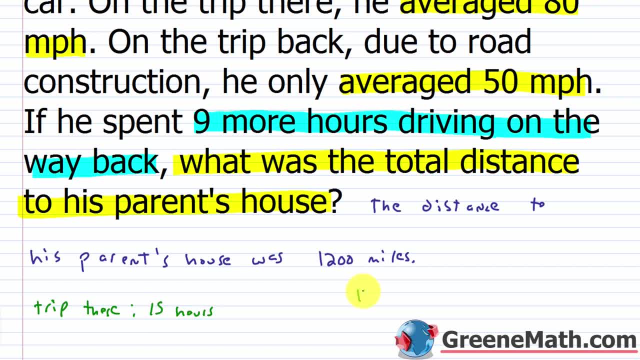 than the trip there. That's how we know we got the right answer. So we would take 1200 and divide it by 50, and this gives us what? Well, this is going to give us 24.. And that's exactly what we want, right. 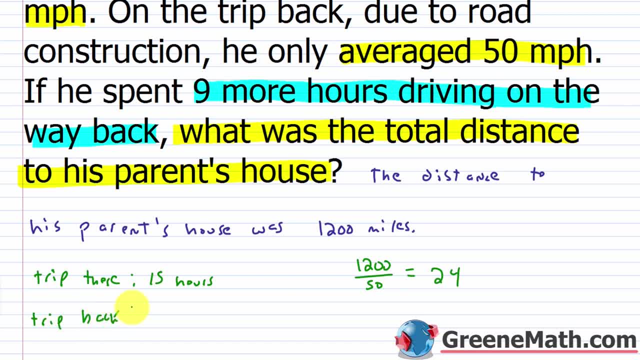 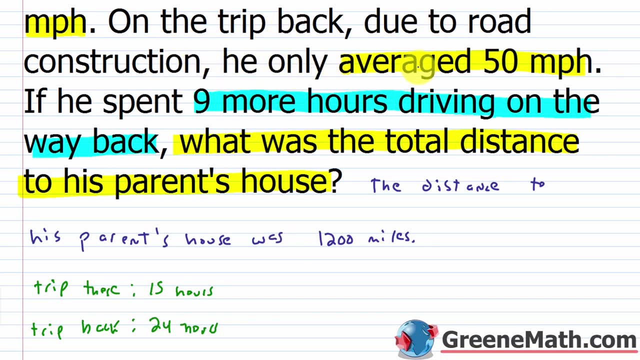 So the trip back is 24 hours And, again, if you look back through the problem, that's what it tells us to expect. It tells us that on the trip back, due to road construction, he only averaged 50 miles per hour. 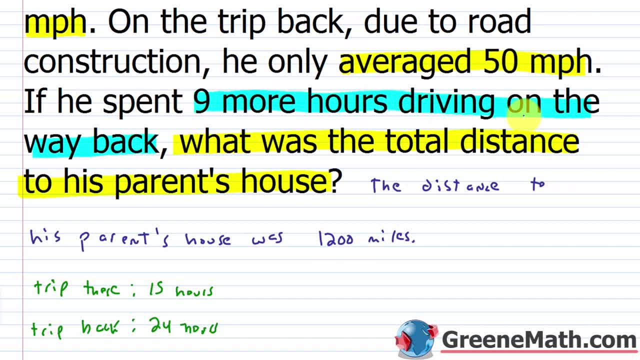 He spent 9 more hours driving on the way back. So on the way back, he spent 24 hours driving. On the way there, he spent 15 hours driving. 24 is 9 more than 15, so we have the correct answer here. 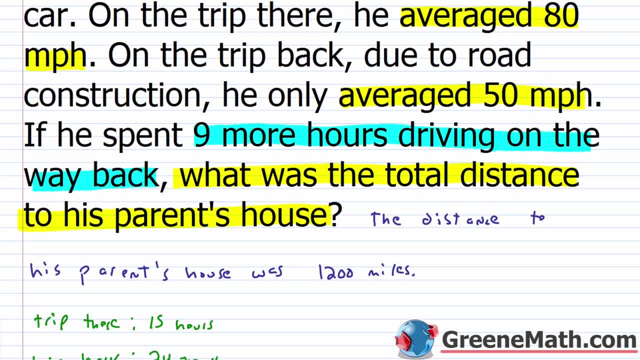 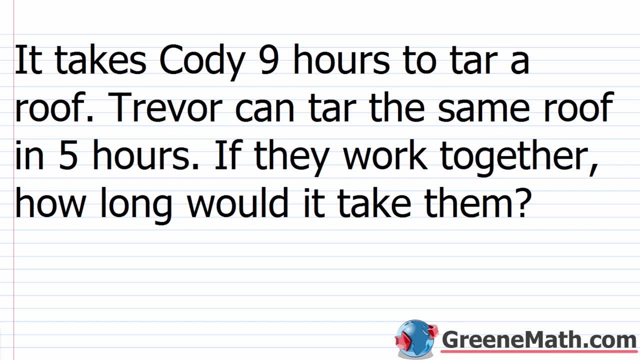 The distance to his parents' house was 1200 miles. All right, let's shift gears for one moment and we're going to look at a problem that deals with rate of work, or work rate. Most of you who have done these type of problems before- 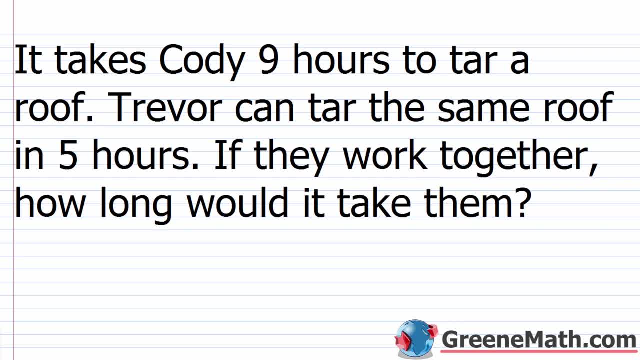 you know they're super easy. They're a little complicated to kind of wrap your head around when you first start doing them, but there's a very easy formula that you follow for them And if you follow that, it's going to be very, very simple. 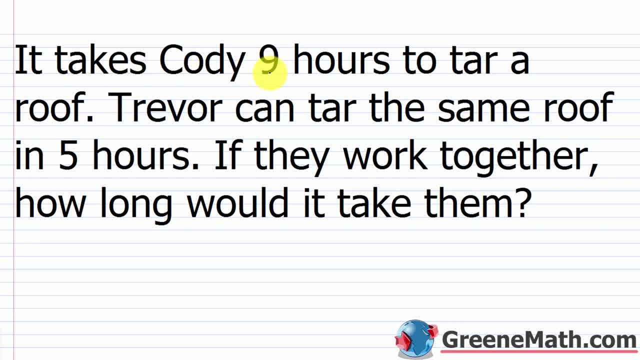 for you to get the answer quickly. So it takes Cody 9 hours to tar a roof. Trevor can tar the same roof in 5 hours If they work together. how long would it take them? So when you work, a work rate problem? 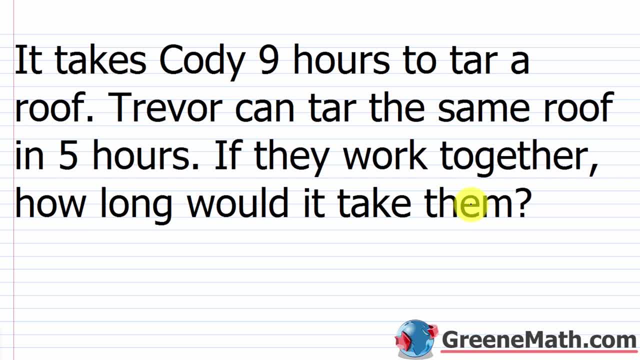 you think about everybody's contribution in terms of one unit of time. So if we're working with hours, our unit of time is hours. So in one unit of time we're thinking of one hour. So for one hour we think about Cody. 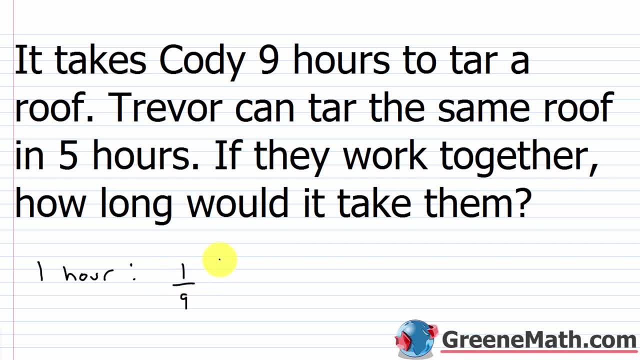 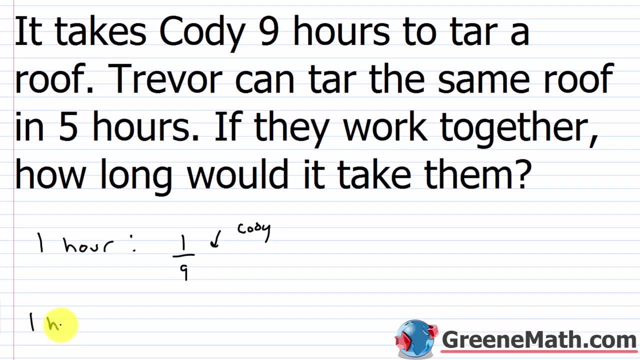 as being able to tar 1, 9th of the roof. Then for Trevor, it takes him 5 hours. So in one hour he's done 1, 5th of the roof. So this is Trevor. So once I have these amounts, 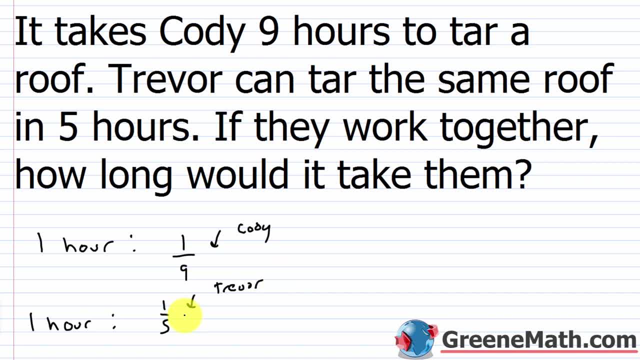 I think about. let's add these two fractions together to see in one hour how much of the job would they do if they worked together. So what is 1 9th plus 1 5th? 9 is 3 times 3,. 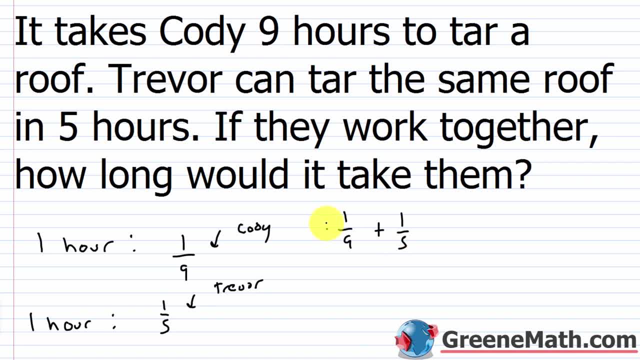 and 5 is a prime number. So I would multiply this by 5 over 5.. I multiply this by 9 over 9.. We'd end up with what? 5 plus 9 over 45,, which is going to give us 14 over 45.. 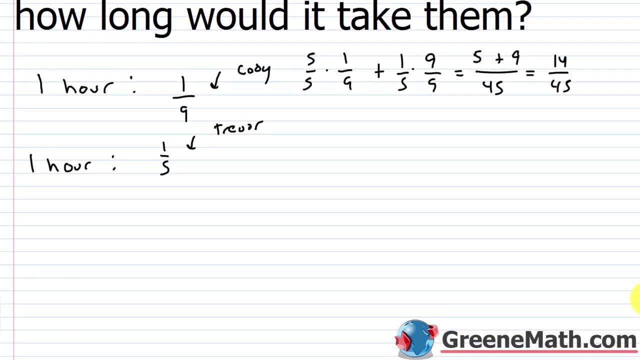 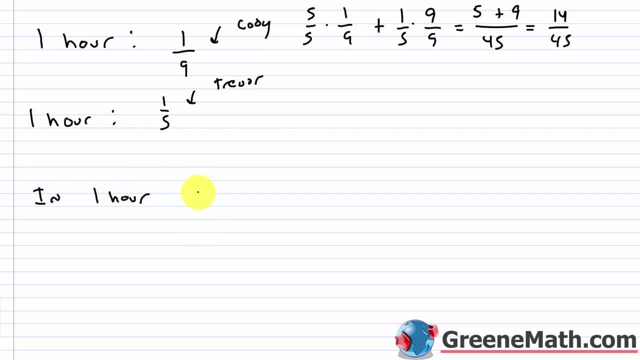 So if I scroll down just a little bit, just get a little room going, we could say that in one hour 14 over 45, this amount of the job is completed if they work together. So in one hour, 14, 45ths of the job. 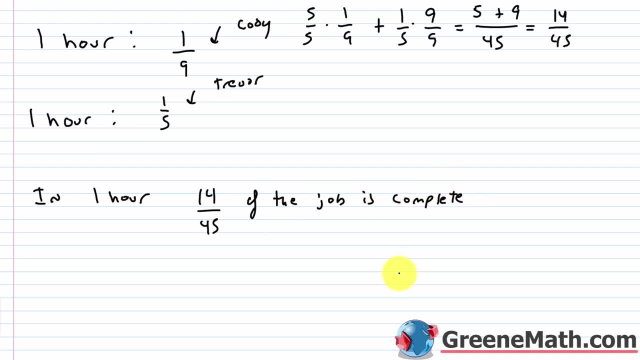 is complete. Now, if we want to see how long it would take to actually complete the job, we could let a variable like x be equal to the number of hours to complete the job. And if you wanted to be more specific on this, 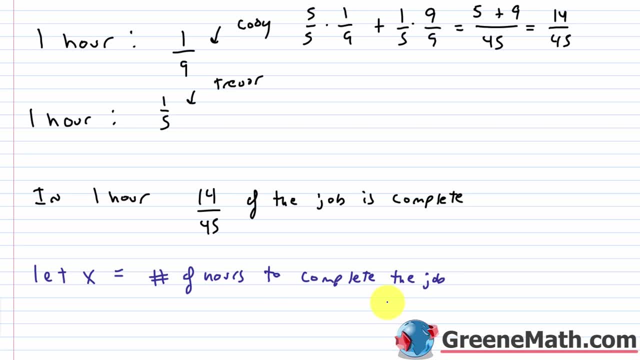 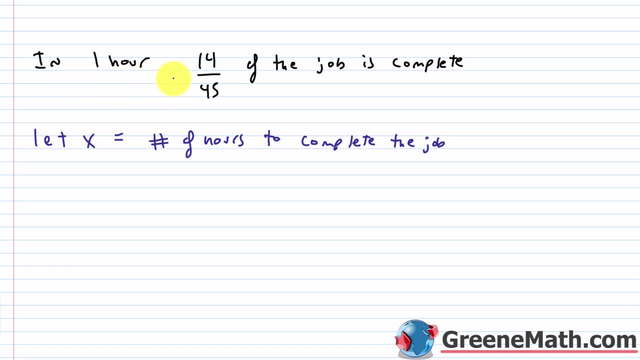 I just wanted to kind of shorten it. you could say the number of hours to complete the job if they're working together. So what would I do? once I have this set up, I have in one hour the amount that working together, they have completed. 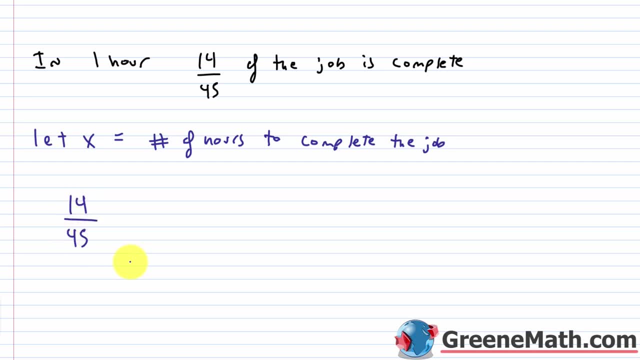 So that's 14 over 45. If I multiply this by the number of hours it takes for them to complete the job, what happens is, this times this will give me one completed job. So once you've set this up- and I know it can be a little confusing. 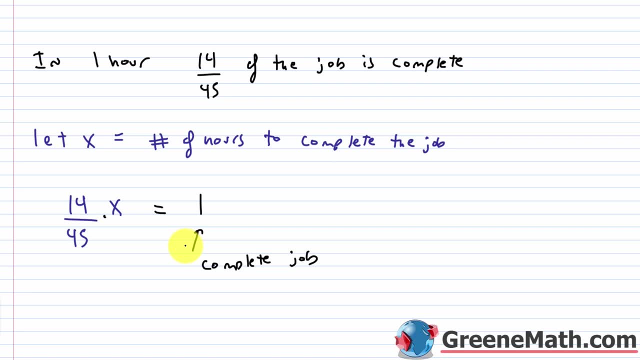 when you first start seeing these, the whole key is starting out by finding out how much they can do together in one unit of time. So in this case it's hours. so we figure out: in one hour Trevor and Cody can do 14- 45ths of the job. 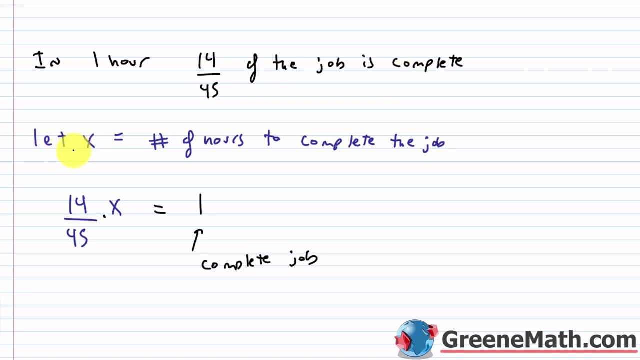 Then we say a variable like x, or you could use y or z or whatever you want, represents the number of hours for them to work together and complete the job. So the amount they complete in one hour, so this is amount completed in one hour. 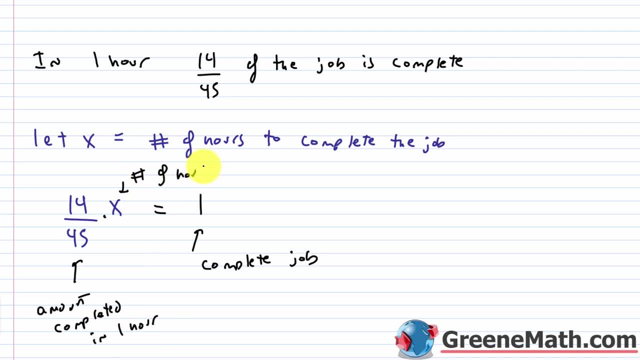 multiplied by the number of hours would be equal to or would give us a complete job. So all we have to do is solve this for x, and that's super easy to do. You're basically going to just multiply both sides by the reciprocal. 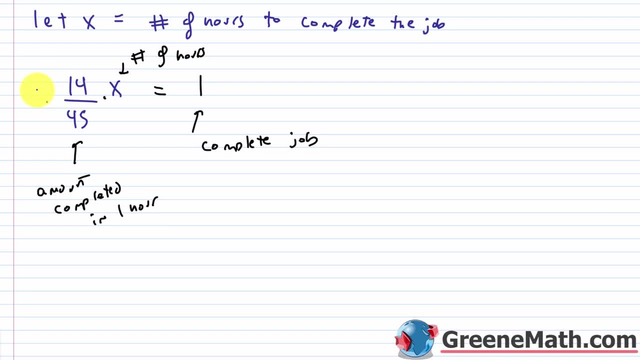 of that fraction. and when we do that, if I multiply this by 45 over 14, and multiply this by 45 over 14, you're going to end up with x is equal to 45 over 14.. So this is how long. 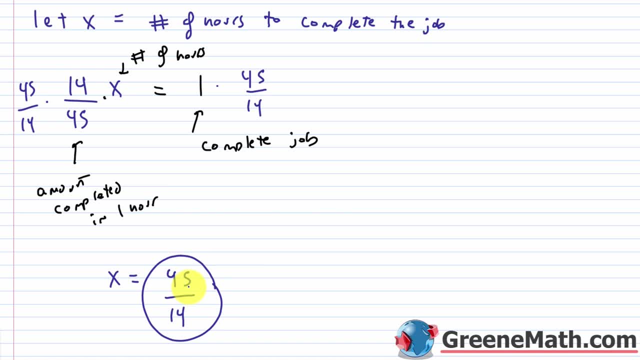 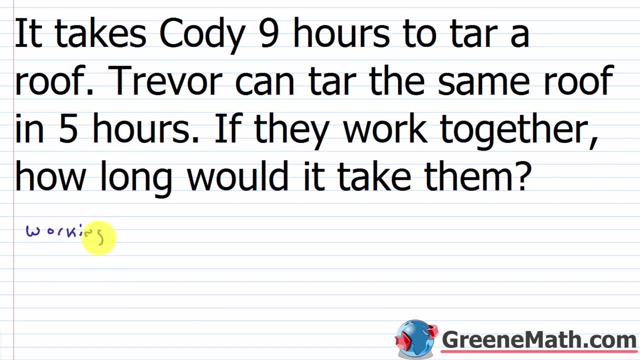 this many hours. right here is how long it takes for them to complete the job if they're working together. So we could say working together it would take 45 over 14, that number of hours to tar the roof. Now, if you do the division on 45. 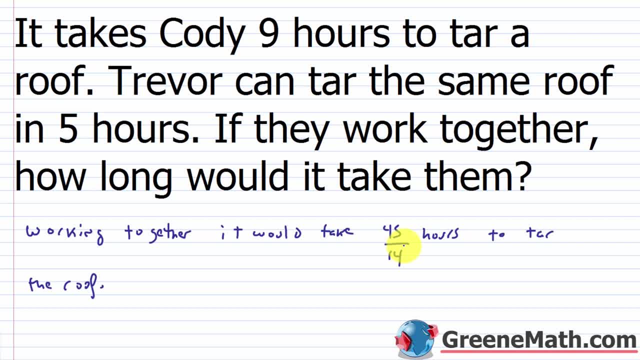 divided by 14, you get kind of a nasty decimal and to not have to round things, I just leave it as a fraction. but it's about 3.21, if you just wanted to estimate about 3.21 hours. 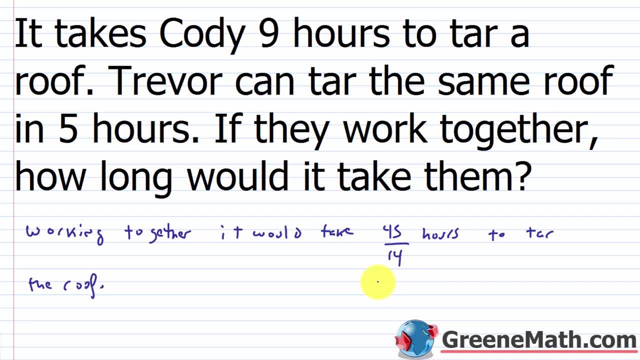 So a lot of teachers would accept that as an estimate. just to make the answer cleaner, but just to be precise, let's say 45 over 14, that number of hours. Now, if you wanted to check this, you could add Trevor's contribution. 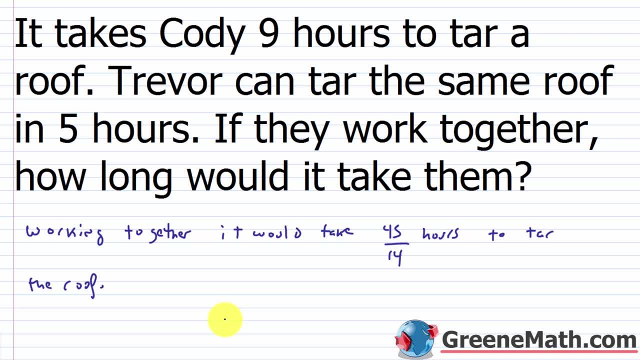 and Cody's contribution and you should end up with one completed job. So Cody's contribution is what He does: 1, 9th of the job in an hour. So if he works for 45 over 14 hours, how much is he going to do? 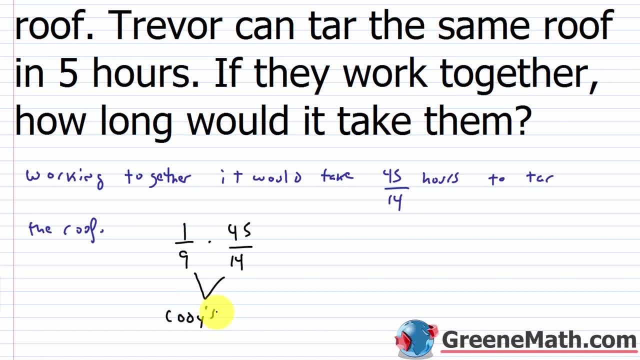 This would be his contribution or Cody's contribution. If we add that to Trevor's contribution, in an hour he does 1, 5th of the job. again he's going to also work for 45 over 14, that number of hours. 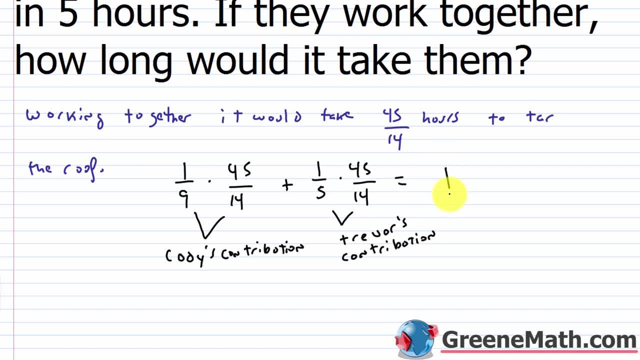 So would this equal 1 completed job? Well, you can look and see that it would. This would cancel with this and give us what It would: give us a 5, so you'd have 5 14ths plus. this cancels with this. 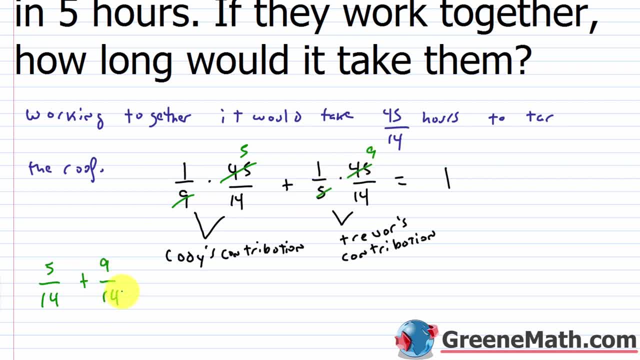 and gives us a 9,. so 9 14ths does us equal 1,. 5 plus 9 is 14,. so this would end up being what This would be: 14 over 14,, which is 1, 1 equals 1,. 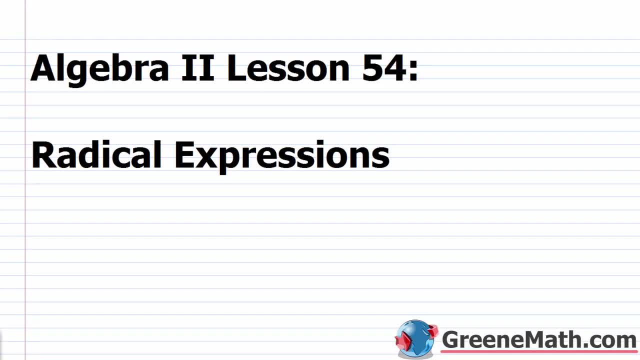 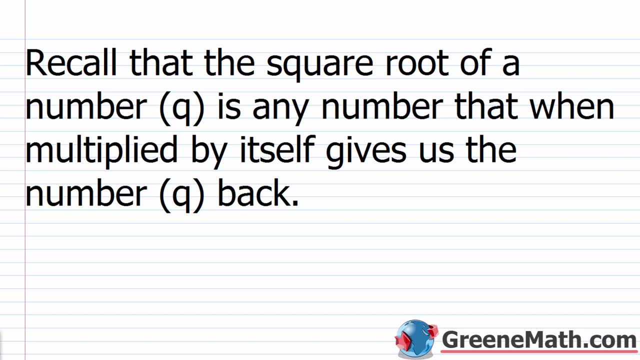 so that equation checks itself out. Hello and welcome to Algebra 2, Lesson 54. In this video we're going to learn about radical expressions. So again we've come to a topic that we learned thoroughly in Algebra 1, and we just need to review here. 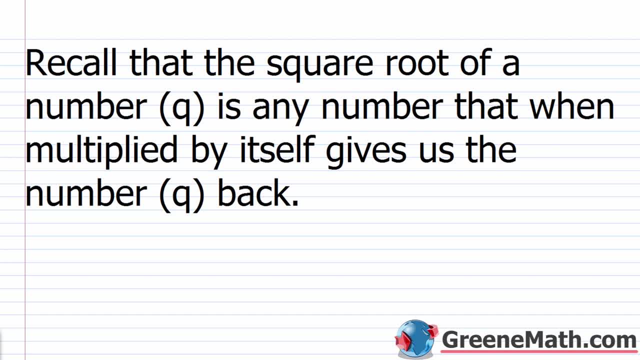 before we get to more challenging material in Algebra 2.. So we're going to start out with the easiest scenario, which is where we deal with square roots. So I want you to recall that the square root of a number, and let's just say that number- is q. 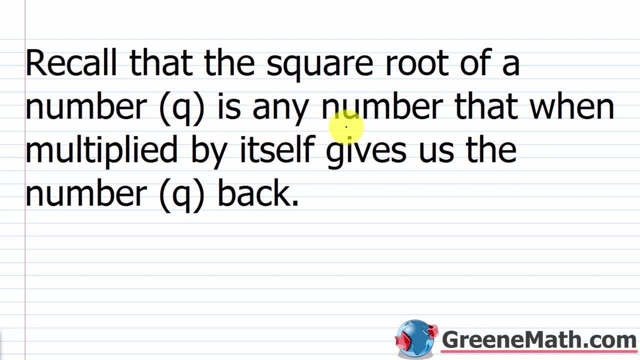 just as a placeholder for now. so this is any number that, when multiplied by itself, gives us the number q. back Now, by using a variable like q, a lot of you will stop and say, well, that doesn't really make a whole lot of sense. 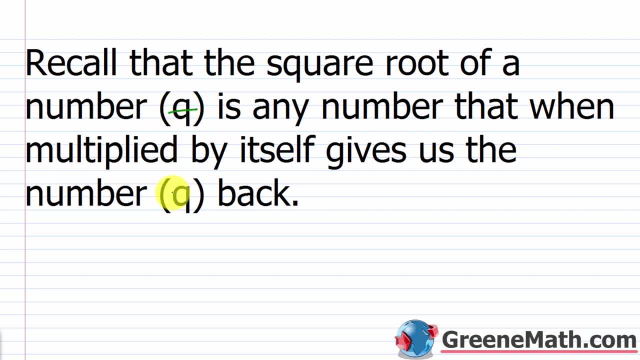 So what you can do, you can just cross q out and you can just pick a number that you know is a perfect square. So, as an example, we know that 4 times 4 is 16, so 16 is a perfect square. 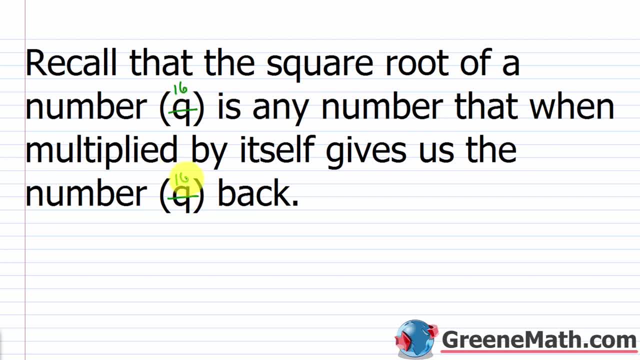 So we can say 16 and 16.. Now if we re-read it, we would say: recall that the square root of a number 16 is any number that, when multiplied by itself, gives us the number 16. back Now we think about 16 as what? 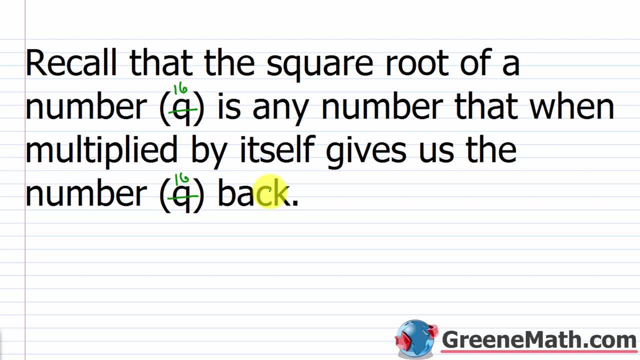 Most of us would say it's 2 to the 4th power. It's 2 times 2, which is 4,, 4 times 2 is 8, and 8 times 2 is 16.. We already know that 16 is 4 times 4,. 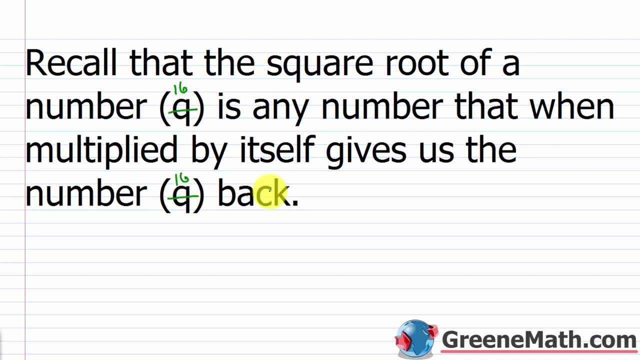 but we might forget that negative 4 times negative 4 is also 16.. So that's where this definition really comes in, where it says it's any number, So it could be more than 1.. So the square root of 16 would be 4,. 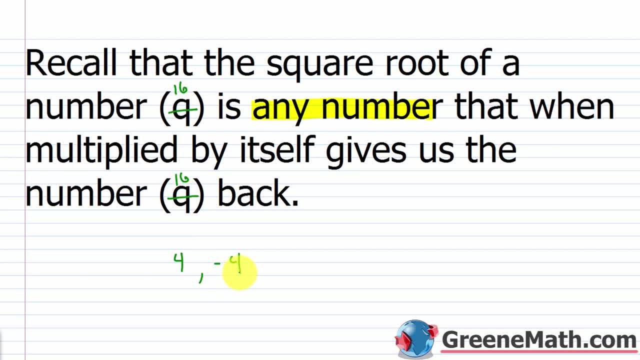 but also it would be negative. 4. Now, when we talk about square roots, we notate the positive square root, or what we call the principal square root, differently from the negative square root, So I would say the square root of 16, like this: 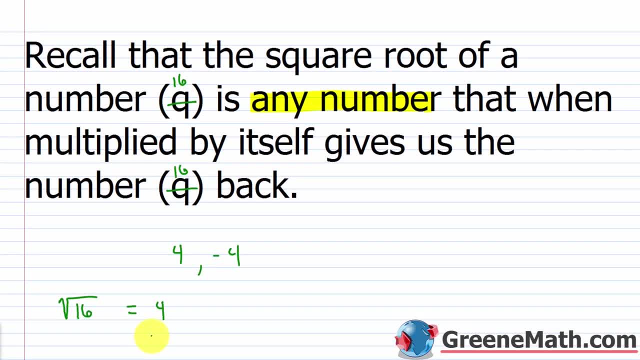 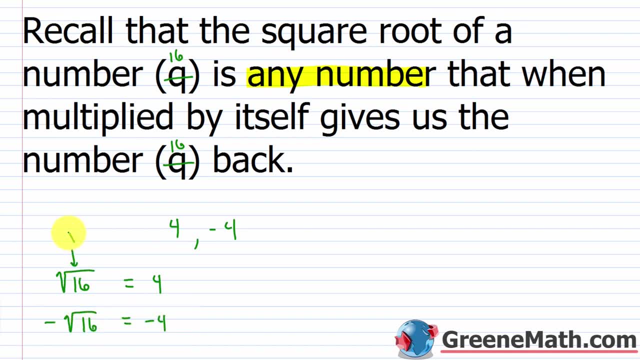 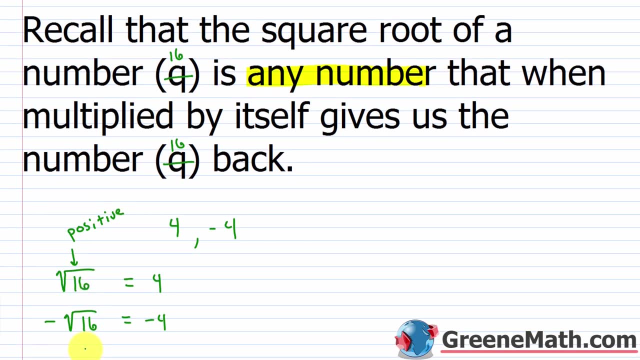 to ask for 4.. I would say the square root of 16, like this: to ask for negative 4.. So this one right here is the positive, or we'd say the principal square root of 16.. Whereas this guy right here because we put that negative out in front. 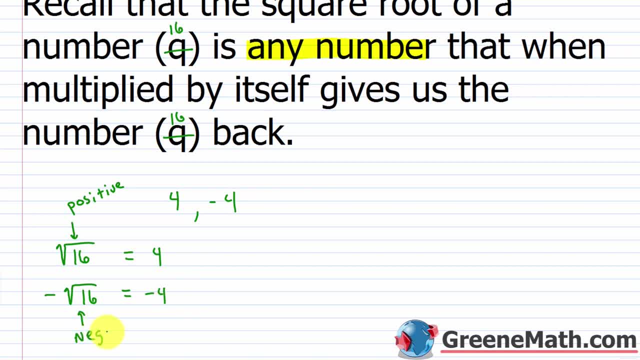 is asking for the negative square root of 16. And the difference between the two is just very, very slight. If I look at this one, I say, okay, well, what positive number, when multiplied by itself, gives me 16?? Well, we know that off the top of our head. 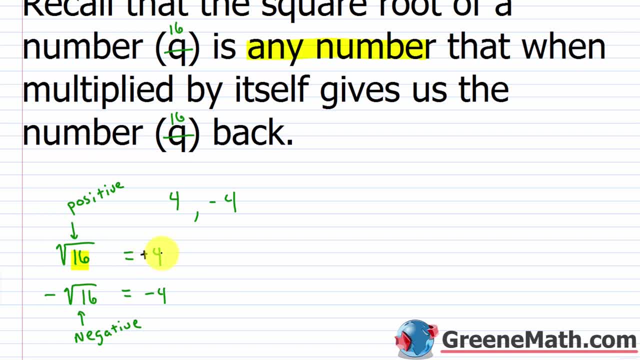 that 4, or more specifically positive 4, times positive 4 would give me positive 16.. When I look at this one, I look at this negative out in front and I say: well, what negative number, when multiplied by itself, would give me 16?. 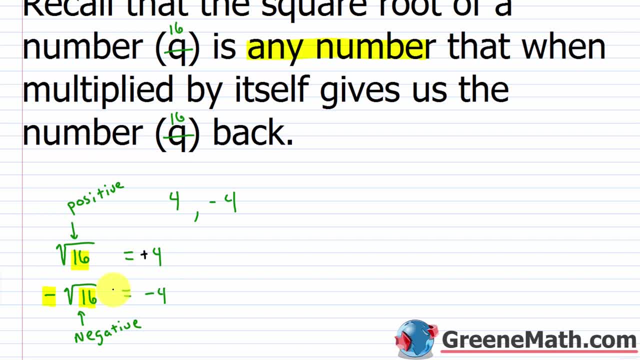 Well, negative 4 times negative 4 would be 16.. So those are the two different notations that you'll run across. If you see something like: what is the square root of 25?? This is just asking for the principal square root. 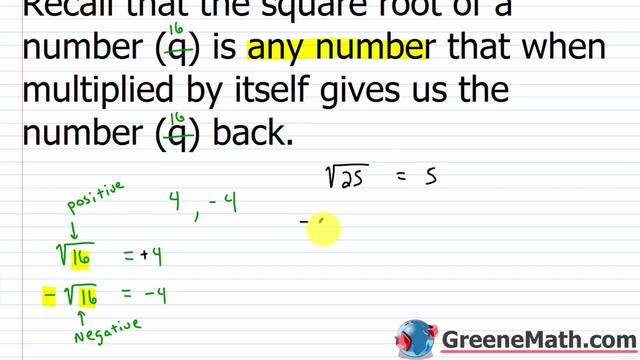 so they just want 5 back. If you see what is the negative square root of 25. like that, they're asking for negative 4.. As we learned back in algebra 1 when we started looking at the quadratic formula, there's a shortcut notation for this. 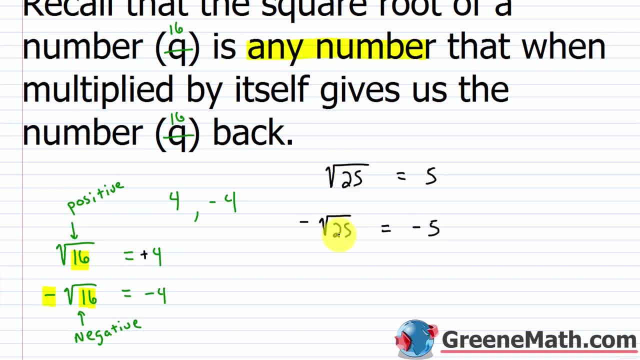 I don't need to separate these two like this. I can just put plus or minus like this in a compact form and then put square root of 25.. This is asking for the positive or principal square root of 25.. It's also asking for the negative square root of 25.. 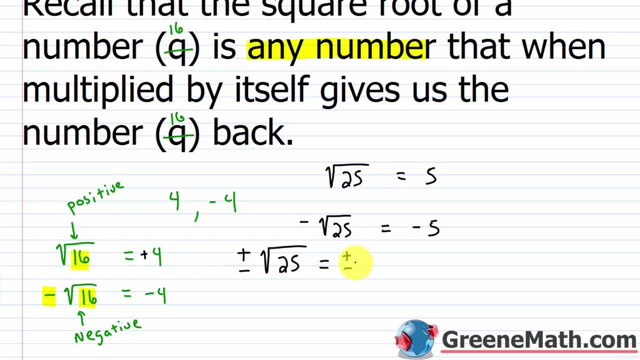 So this I can put as equal to plus or minus 25.. So I'm accounting for both possibilities. The positive square root of 25 is 5.. The negative square root of 25 is negative 5.. So this is again just a more compact way. 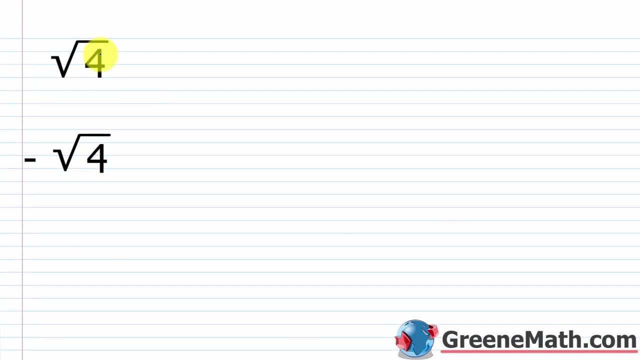 to write things. So let's just look at a quick example here. So we have the principal square root of 4.. So that's asking for what positive number, when multiplied by itself, would give me 4.. All of us know that would be 2.. 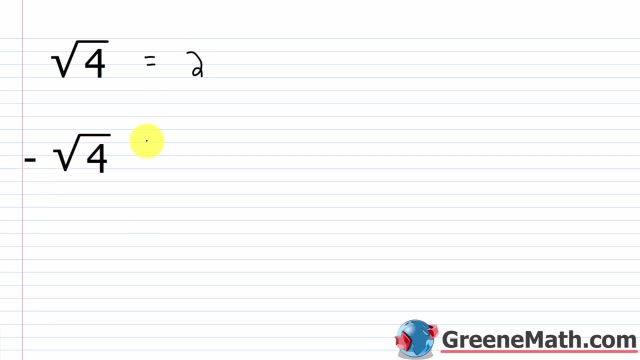 2 times 2 is 4.. Now, with this one we have the negative square root of 4.. So we're saying: hey, what negative number, when multiplied by itself, would give me 4 and that's negative 2.. Now again, if you want to practice that more compact notation, 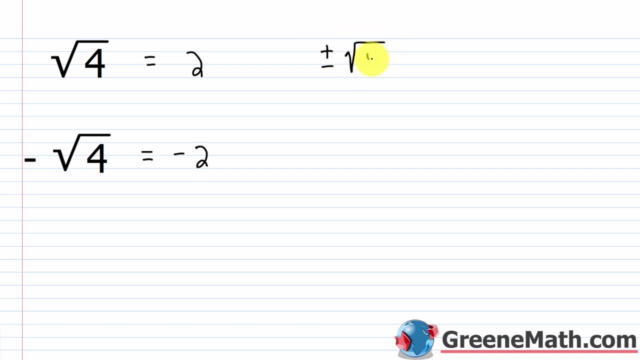 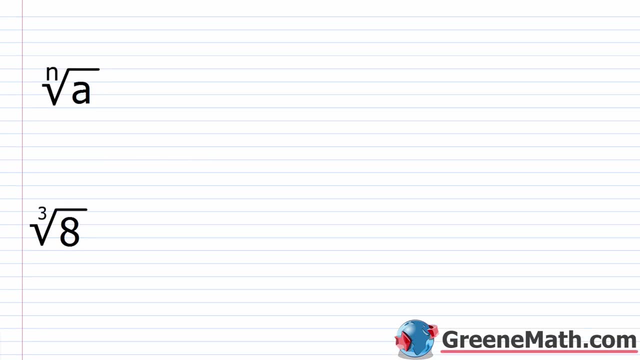 you could say plus or minus the square root of 4, and that's equal to plus or minus 2.. Alright, so let's look at something with higher roots now. So we should know at this point that, in general, when we see a square root, 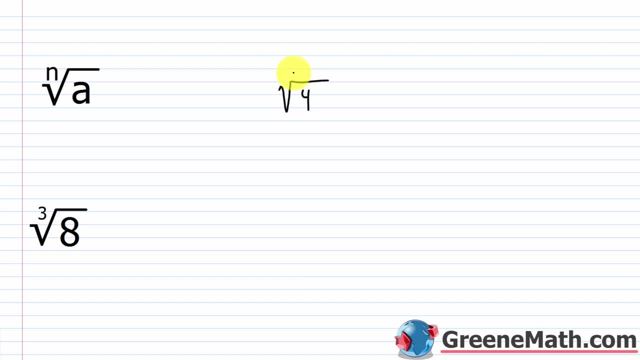 it's really what If I have the square root of 4 like this, it's missing a number there that we normally display for higher roots, because square roots are so common- Square roots are so common that we just leave that off. but that number that's missing is a 2.. 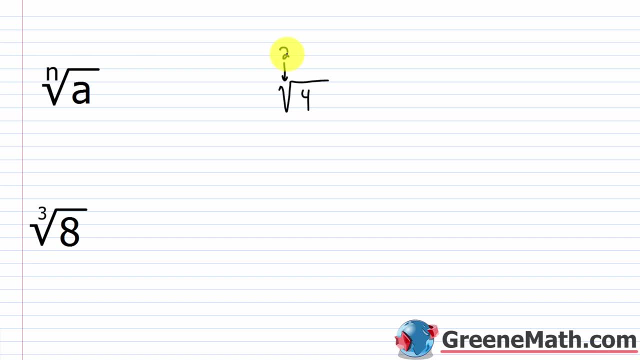 That 2 is known as the index or the order. So in this generic example here we have the nth root of a. So right, here, this is the index, or you could say it's the order. This a right here. this is known as the radicand. 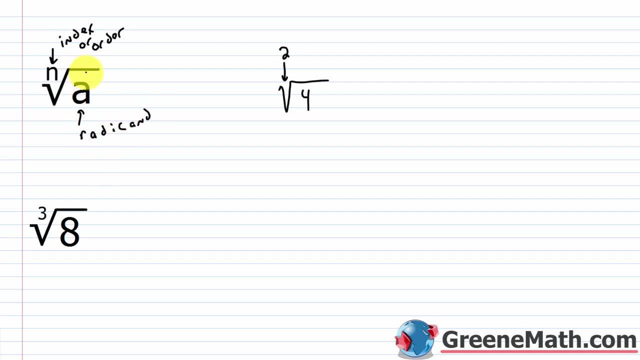 that's the value that's under the radical symbol. so we'll label this, we'll say this is the radical symbol and the whole thing. if I looked at everything involved here, that's just known as a radical. So if I say, hey, you got this radical. 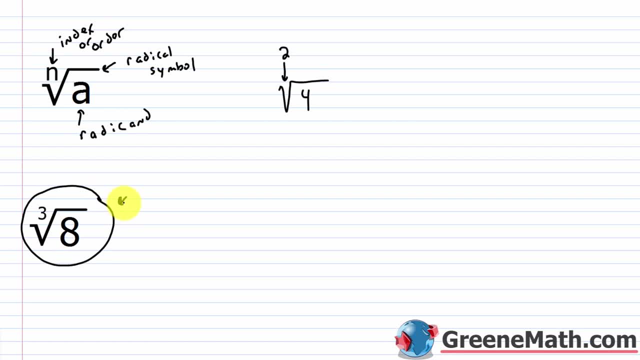 I'm talking about everything. So this whole thing right here is a radical. So, again, when we see square roots like the square root of 4, we don't display an index or order because it's understood to be 2.. So if I wanted the square root of 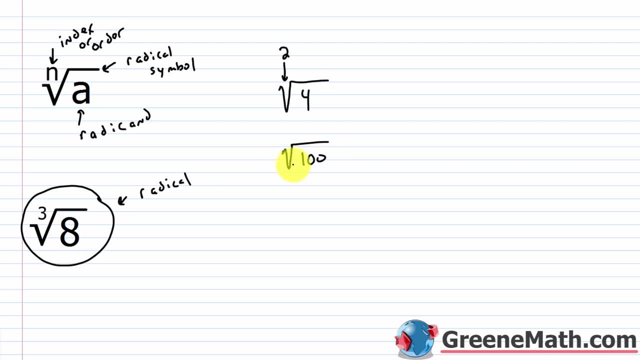 let's say 100. I would write it like that. Now it wouldn't be incorrect if I wrote the square root of 100 like this and put a 2 here. it's just not common to see that Now as we move into higher level roots. 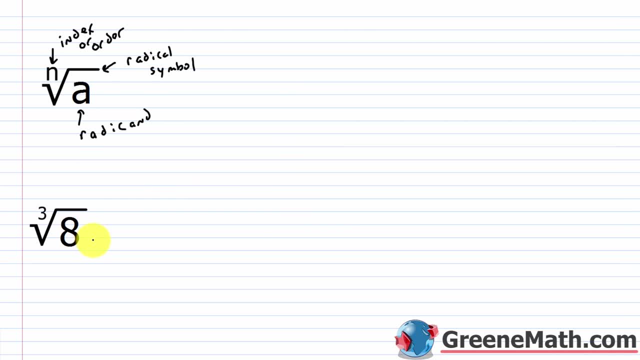 we see something like this. I'm going to start out with something known as a cube root. So the index is a 3, this is my index and my radicand is an 8. so this is my radicand and before we think about this, 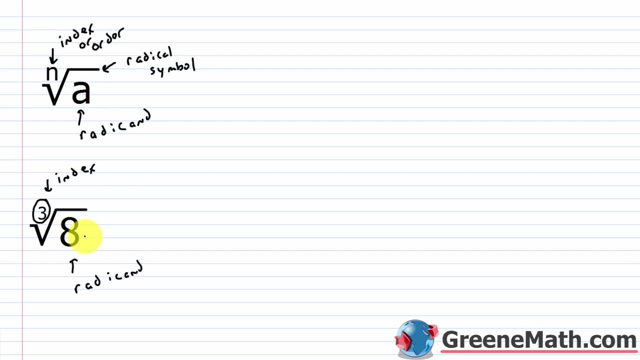 let's think about the square root for a second. if I want the square root of 4, I'm thinking about what number, or numbers, when multiplied by itself, is going to give me 4.. Now, the reason I'm doing that is because, if I think about the square root of 4, 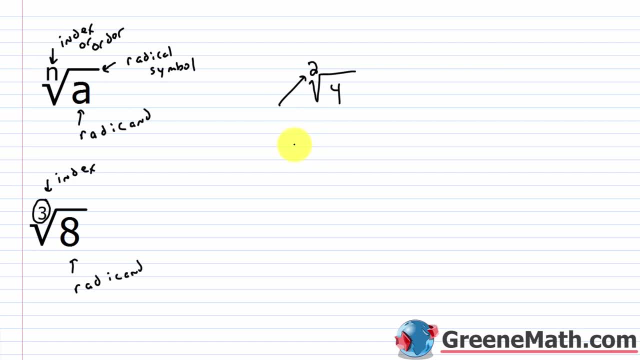 again, this is a 2. so I'm saying, hey, what number multiplied by itself twice is going to give me this value here? When I look at a cube root now, I'm thinking about a number that, when multiplied by itself 3 times, because the index is a 3- 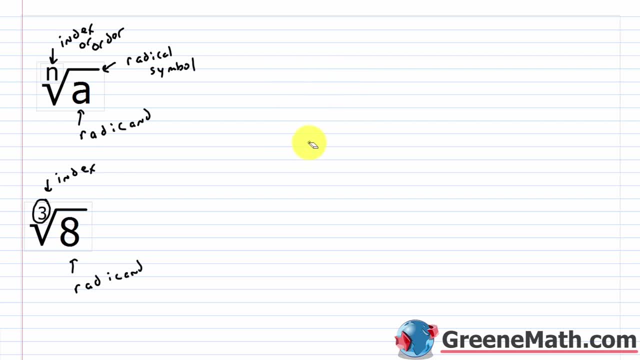 is going to give me that radicand back. So, with the cube root of 8, with the cube root of 8 again, I'm looking for a number that, when multiplied by itself 3 times, would give me 8.. Now, for most of you would know, this is 2.. 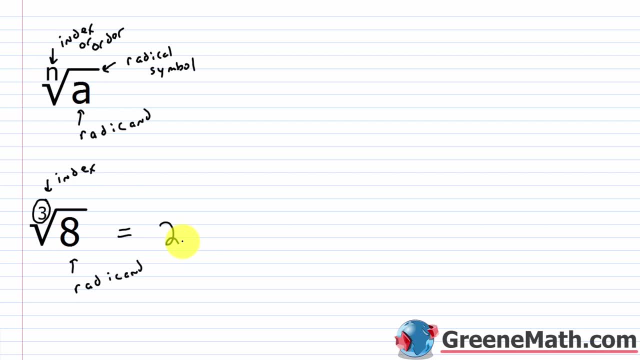 2 times 2 is 4, 4 times 2 is 8. so that would be your answer there. But if you didn't know something like that, you can always go back to your factoring. you can say: I know, 8 is what it's 4 times 2. 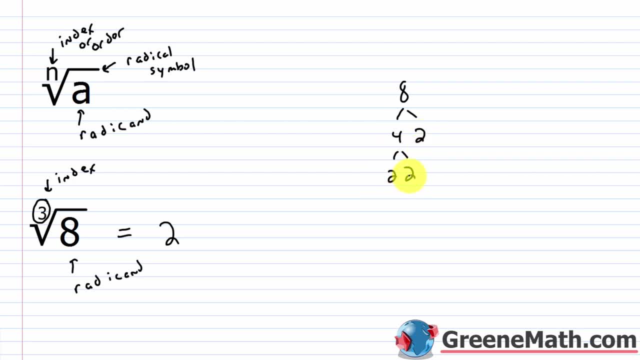 and I know 4 is 2 times 2. these are all prime factors. so I know it's 2 times 2 times 2 or 2 cubed. so again, the cube root of 8 is 2.. Now you'll notice that. 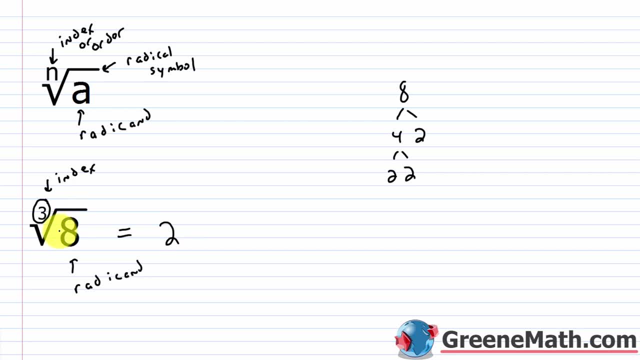 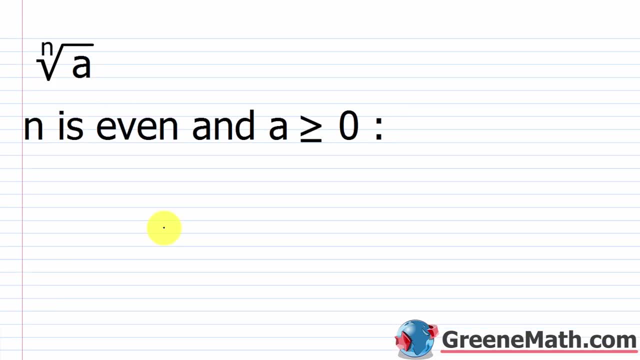 I didn't give you 2 sets of notation for this one here, and that's not because it's a higher root, it's because this index is odd. So I want to just cover some rules that you need to know, something you want to definitely jot down. 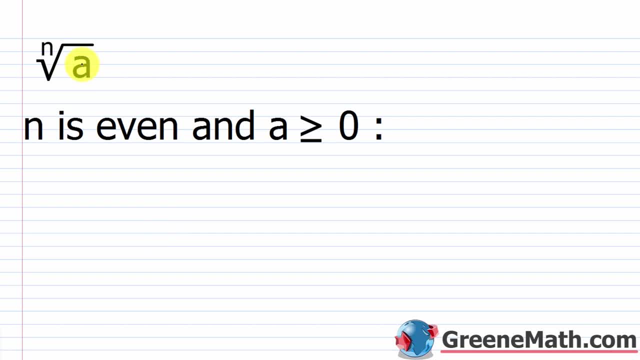 so if you see something like the nth root of a- and I know we don't like working with generic examples, but just something you can substitute in to your given example- you say that you have the nth root of a. n is even so. n is, let's say, 2: 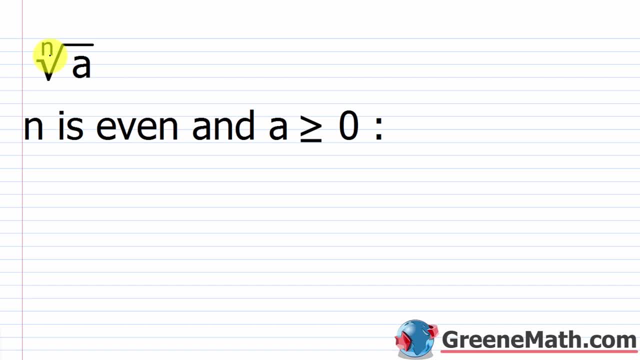 or it's 4, or it's 6, or it's 8 or it's 10, something that's divisible by 2, and then also in this scenario, a is greater than or equal to 0. so basically, a is not a negative value if this occurs. 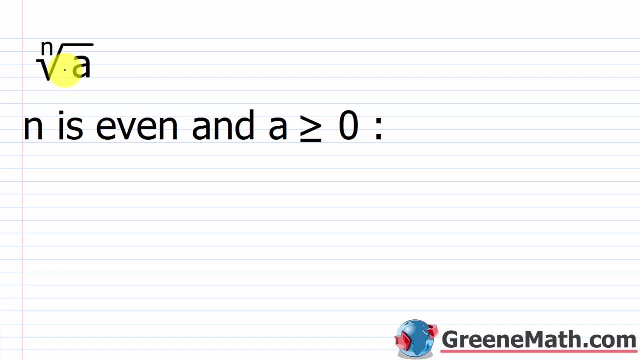 we're going to have 2 sets of notation, just like I showed you. so you're going to have the nth root of a like this: this is your principal root. then you have the negative of this. so negative nth root of a: this is your negative. that's the negative root. 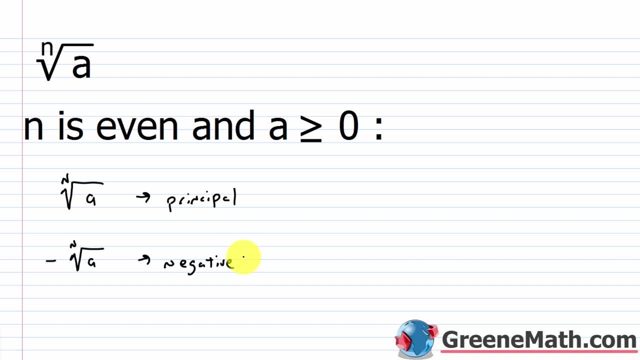 so in that scenario we had, let's say, the square root of 4. for example, square root of 4 is 1, that's 2, that's your principal root. then you have the negative square root of 4, which is negative 2. but again, it's not just with the square root. 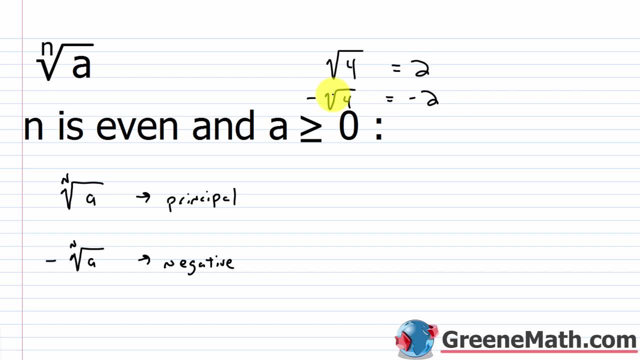 it could be a 4th root or an 8th root, something easy to do. let's say we had the 4th root of 16, so the 4th root of 16. many of you know that 2 to the 4th power is 16. 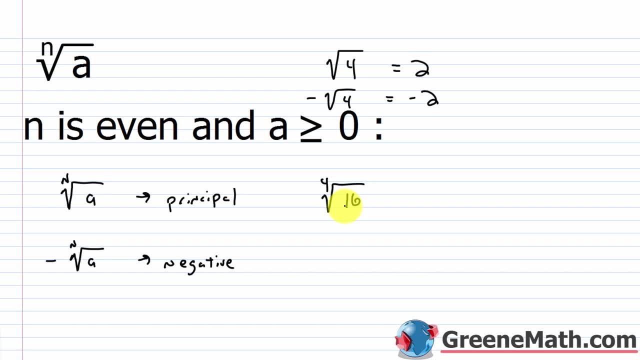 2 times 2 is 4. 8 times 2 is 16. so we know this would be 2, but then you'd also have to account for the negative 4th root of 16. this would just be negative 2, and if I multiply negative 2 by itself 4 times, 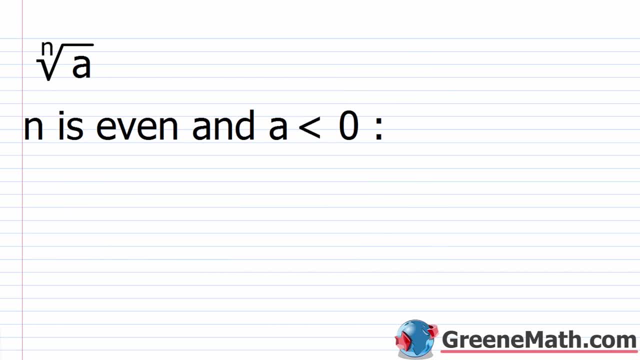 I would get positive 16 as a result. alright, the next scenario I want to talk about: if we have the nth root of a and n is even and a is less than 0, so now a is a negative value. so you'll recall this from algebra 1, where we said: 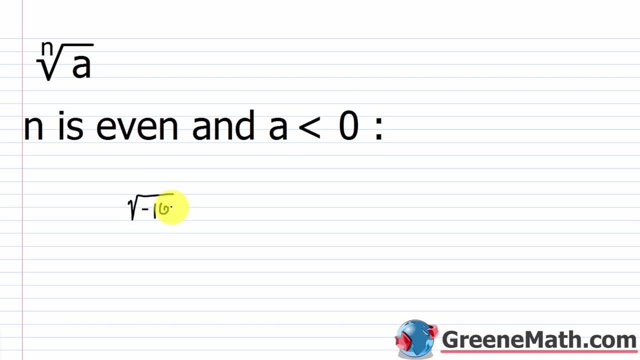 the square root of I don't know, let's say, negative 16. what happens here? well, it's not a real number and we're going to learn how to deal with this in algebra 2. we didn't talk about it in algebra 1, but we will have a way to evaluate this. 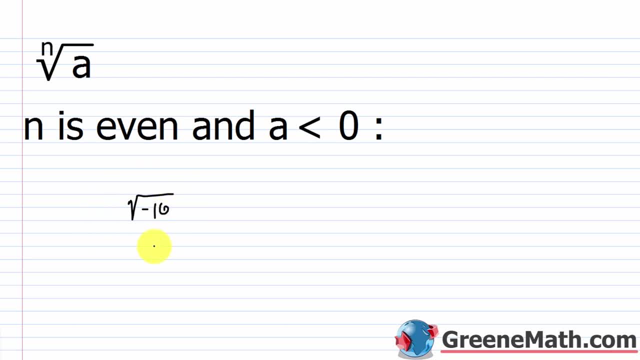 using something known as imaginary numbers. but we haven't gotten to that yet, so for right now, we just say that this is not real. this is not a real number. so again, if n is even so, 2,, 4,, 6,, 8, 10,, 12, whatever it is, 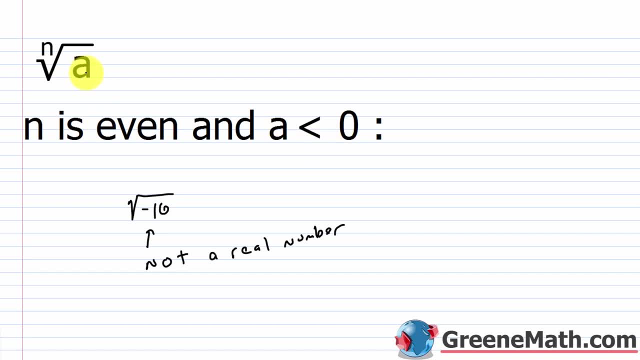 and a is less than 0, a is a negative value, then you're going to write that it's not a real number. so let's say you have the 4th root of, let's say, negative 625. again, this is even this is negative, so it's not. 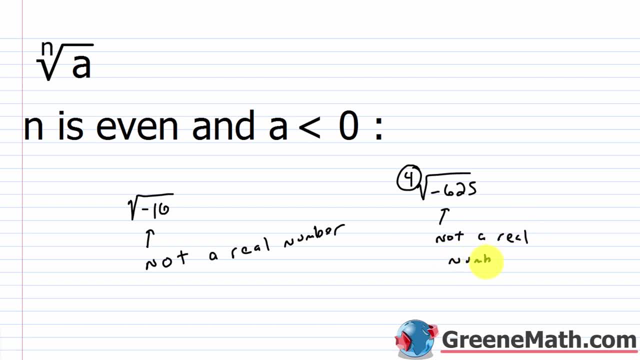 a real number. alright, the final scenario: if you have n, that's odd, x is odd, a can be whatever. it can be positive, it can be negative, it can be 0, it can be whatever you want it to be. you're only going to have one root. 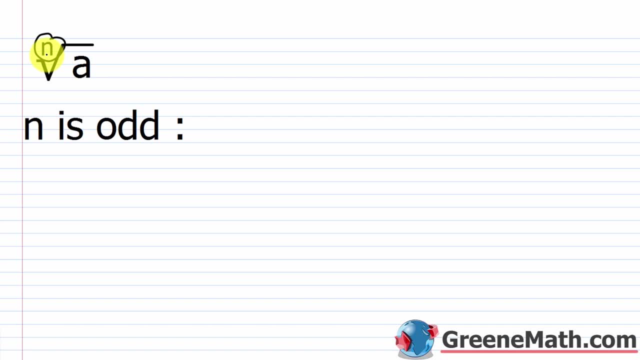 and the reason for this deals with the rules for positives and negatives. if I multiply a negative by itself an odd number of times, I get a negative. so if I had something like, let's say, the cube root of negative 8, so what number when multiplied by itself? 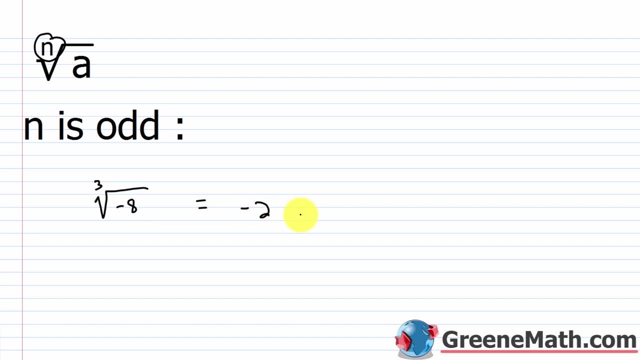 gives me negative 8. well, that's negative 2. negative 2 times negative 2 is positive 4. then positive 4 times negative 2 is negative 8. just keep in mind that you are allowed to have a negative radicand if this guy. 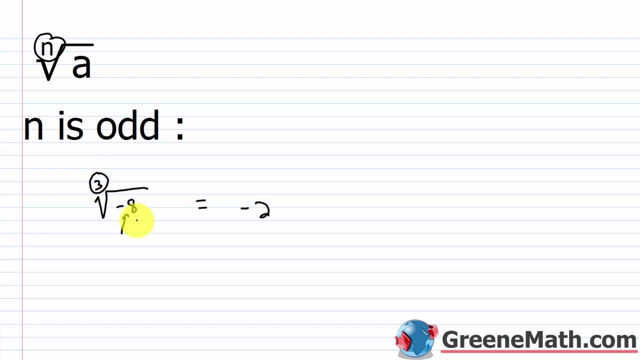 is odd. it's just the case where you can't have a negative radicand when that guy is even so a lot to kind of throw at you, especially if you didn't learn this back in algebra 1. it's just one of those things where 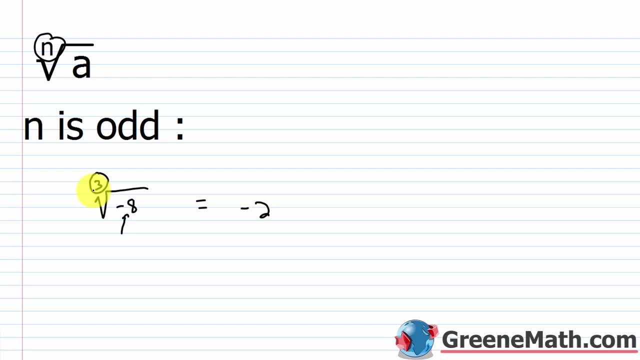 you just have to practice enough and it's something you're going to have down pretty much right away. alright, so let's just take a look at some really easy examples. so we've seen this already. if I had the principal square root of 25, we know that would be what. 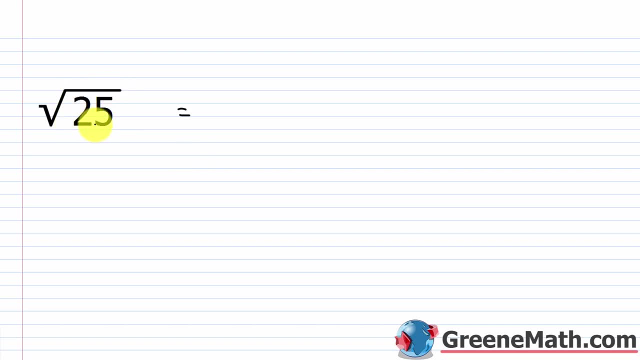 I'm just asking for a positive number that, when multiplied by itself gives me 25. we know that would be 5. then what about the square root of negative 25? now again, if I have a negative radicand and I have an index, that's even. 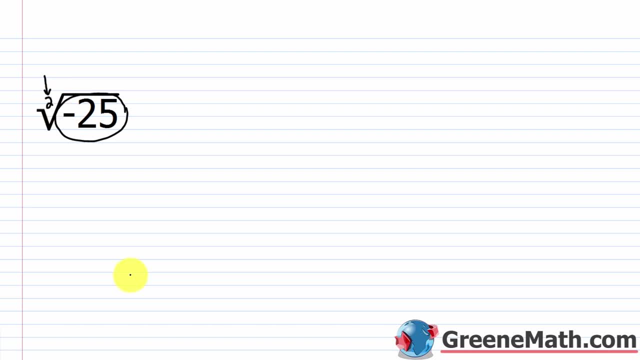 in this case, the index isn't shown, but it's an invisible index of a 2. what happens here? this is not a real number. this is not a real number now. don't get this confused with what we're going to see now. here we have the negative square root of 25. 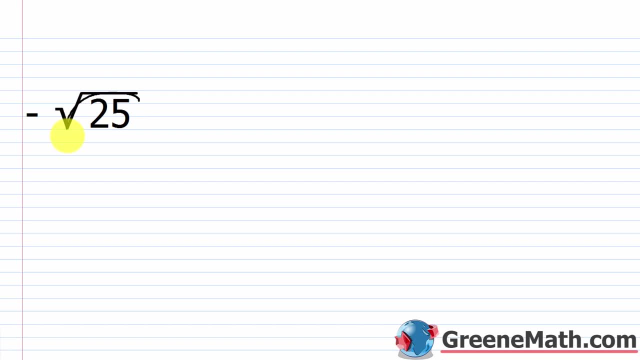 underneath the radical symbol. I have a positive value, so I'm ok, this is positive. it's the negative outside that's telling me: hey, I want the negative square root of 25. that's a big source of confusion. so make sure you understand the difference between the two. 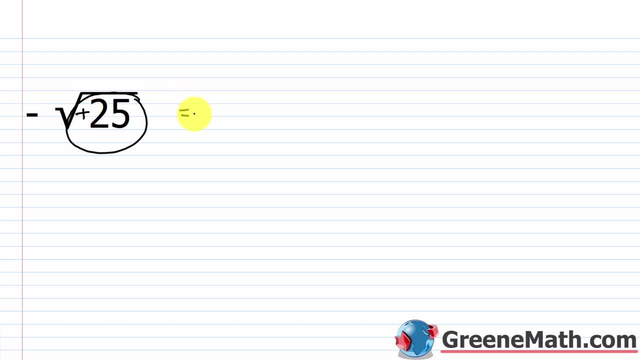 the negative square root of 25 is just asking for what negative number, when multiplied by itself, will give me 25 and that's negative 5. negative 5 times negative 5 is 25. alright, for the next example, we have the principal fourth root of 81. 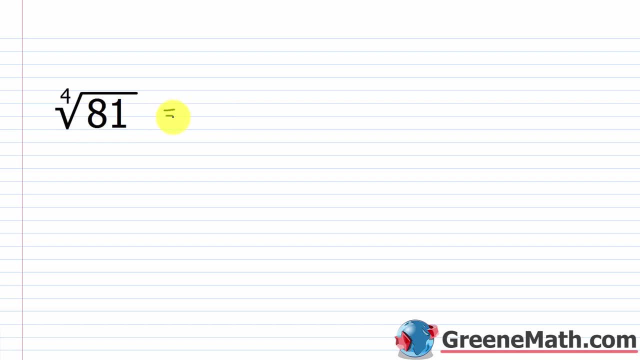 so we're asking for what positive number, when multiplied by itself 4 times, is going to give us 81. well, some of you will know right away that's 3. if you didn't again, you can use a factor tree. so take 81 and break it down. 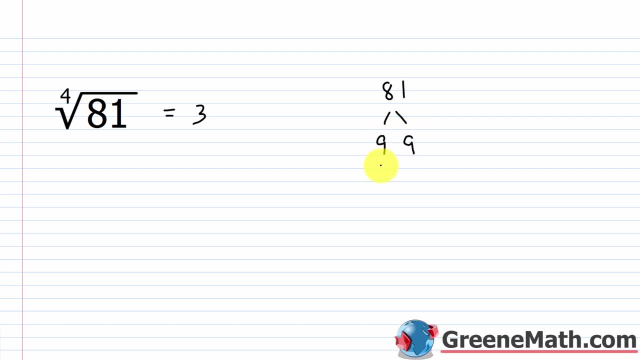 most of you will know that 81 is what it's 9 times 9. 9 is 3 times 3. so just a quick factor tree will show you: 3 times 3 times 3 times 3, or 3 to the fourth, power is 81. 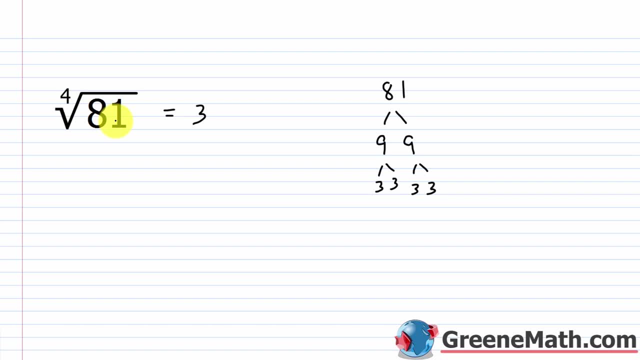 so that means, if I'm looking for a positive value that, when multiplied by itself 4 times, is going to give me 81, we know that's going to be 3. alright, what about the cube root of negative 64? because this index is odd, I know I'm going to have. 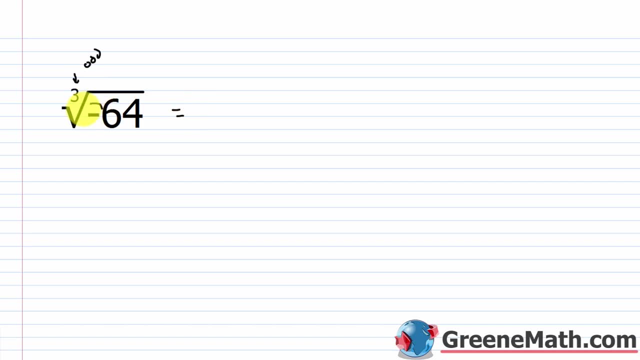 one answer, and I know that the negative is allowed. this is ok again, because this is an odd index. a negative times, another negative times, another negative, or 3 negatives or an odd number of negatives in general will produce a negative. so all you got to ask yourself is: 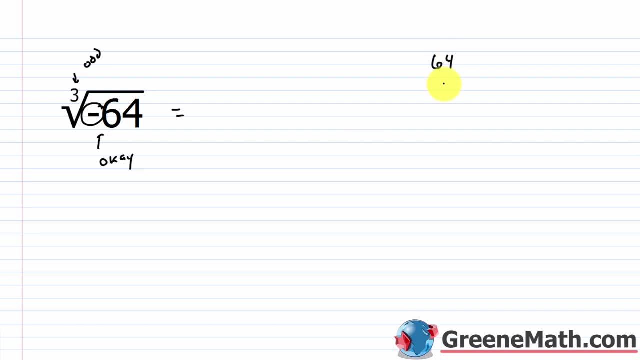 take 64. forget about the negative. for a second: 64 factors into what it's 4 times 16. 16 is 4 times 4, so without going into 4 as 2 times 2, I know I have 4 times 4 times 4 or 4 cubed. 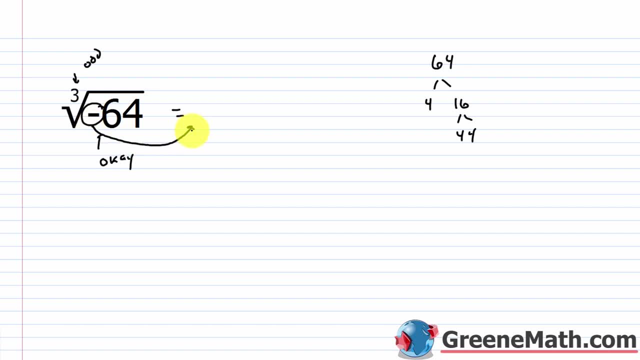 that gives me 64. all I got to do is just drag this negative over here and say this is negative 4 because the negative times, the negative times, the negative will give me a negative back. so negative 4 times, itself 3 times, will give me negative 64. 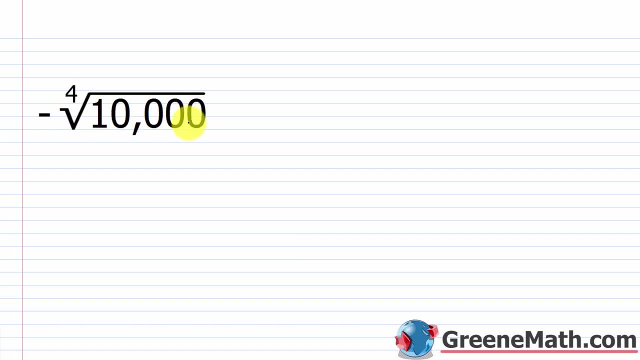 all right. for the next one, we have the negative 4th root of 10,000. so what are we looking for here? we're looking for a negative number that, when multiplied by itself 4 times, is going to give us 10,000 now. so I'm just going to put a negative. 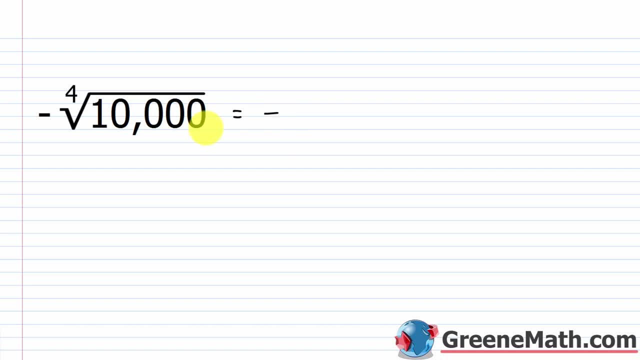 out in front because I could just forget about it now. now I just think about 10,000. 10,000 is a power of 10, so it's really easy, right? it's a 1, followed by 1, 2, 3, 4, 0's. 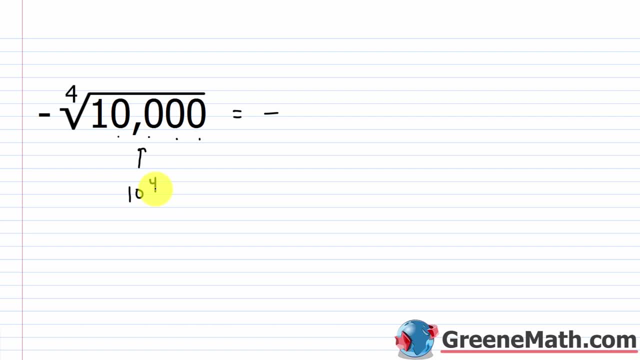 so that means it's 10 to the 4th power. so the 1 way I get that is, if I'm evaluating something like this 10 to the 4th power, you write a 1 and you follow it by this mini 0. so this is 1, 2, 3. 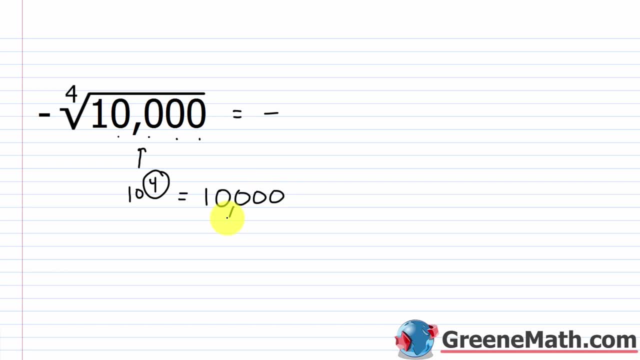 4. so kind of a cool trick if you don't know that, so I automatically know that if 10 to the 4th power is 10,000, the 4th root of 10,000. forget about the fact that it's the negative. 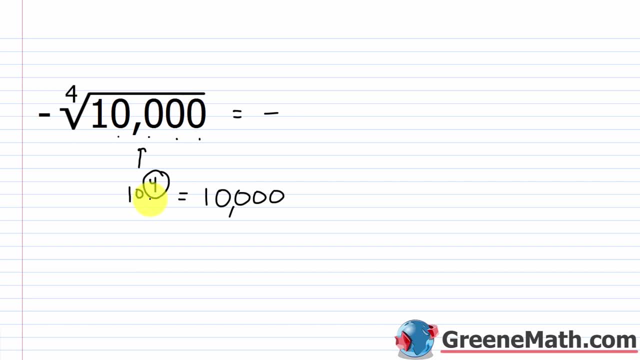 4th root. we've already accounted for that. the 4th root of 10,000 would just be 10, so we just put negative 10 here as our answer. negative 10 times negative 10 is 100. 100 times negative 10 is negative. 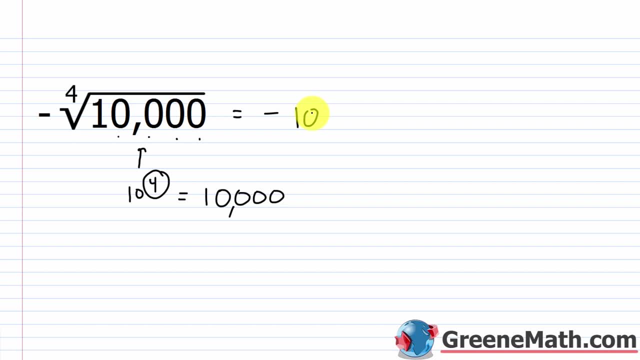 1000 negative. 1000 times negative 10 is 10,000. alright, let's take a look at another one. let's say you saw the cube root of negative 125. so again, if I'm thinking about something like this, this is negative. 3 negatives makes a negative. so I just 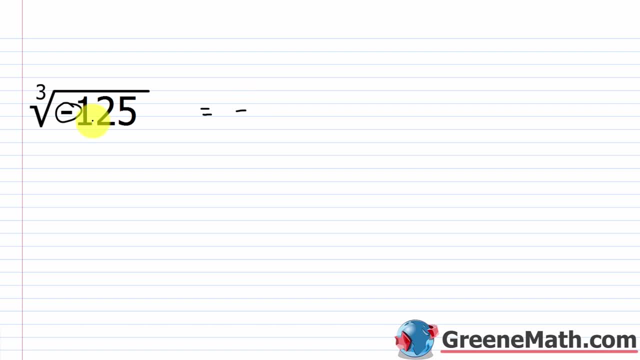 start out with putting a negative there. then you can just forget about it and you can say, okay, well, 125, 125 would factor into what 25 times 5? 25 is 5 times 5, so 5 cubed would be a 125. so what I'm looking for? 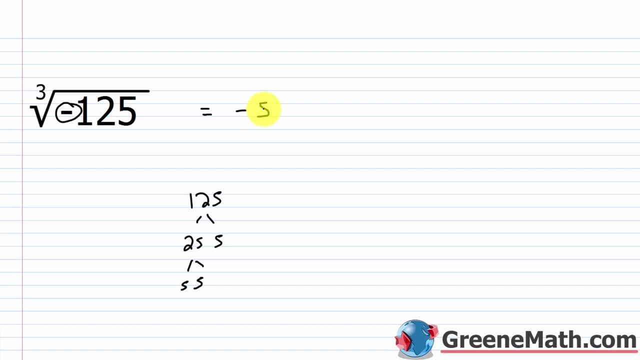 here is negative 5. negative 5 times negative. 5 is 25, 25 times negative, 5 is negative: 125. alright, last one, we have the principal 4th root of negative 16. so again, I have a negative radicand and I have an even index. 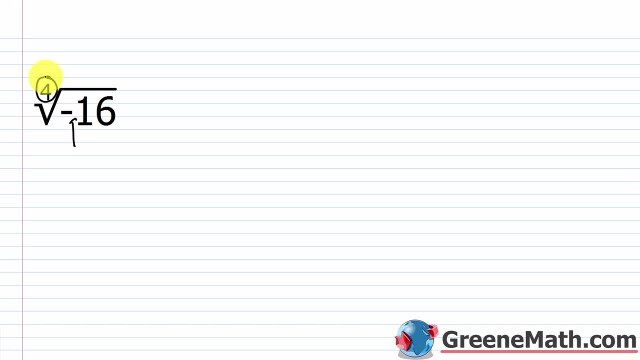 so when that happens, we don't have a real number. this is not a real number and again, the reason for that is I can't take a negative and multiply it by itself 4 times and end up with a negative. right, it's going to give me a positive. 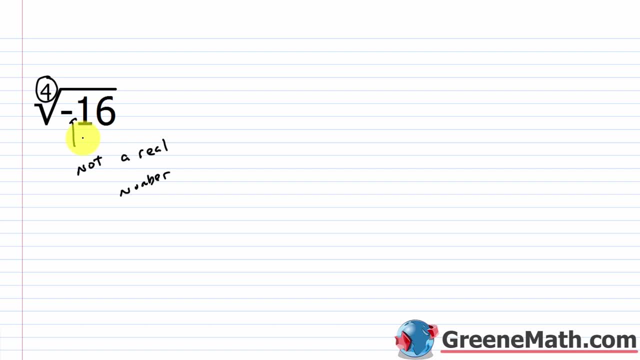 an even number of negatives will always give me a positive, and so that's why this value doesn't exist using real numbers. alright, let's take a look at another rule. that's pretty time saving for us if we have the nth root of a to the nth power. 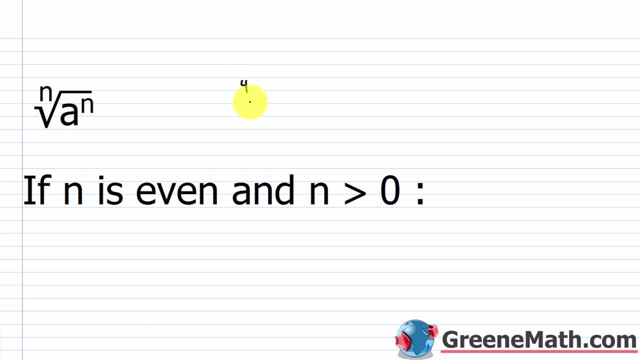 so something like if you had the 4th root of, let's say, 2 to the 4th power, what would you guess would happen there? well, you know from your studies of algebra 1- or hopefully you remember- that this ends up canceling with this and you're. 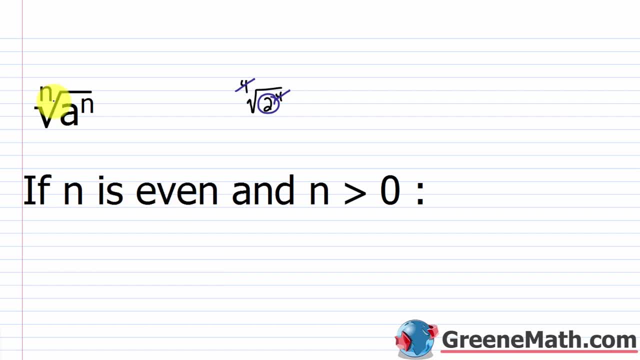 left with this right. so if n is even, so, in other words, if this is even and this is even, they're the same value and n is greater than 0. so even and greater than 0, then what we're going to find is we have the nth root of a to. 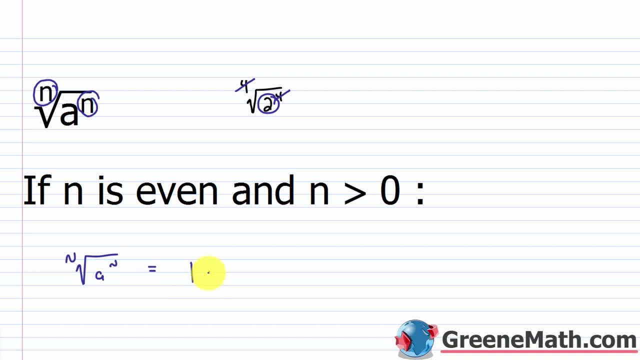 the n, we'll say this is equal to the absolute value of a. so as an example, let's just say we took something like 5, so we take the 6th root of 5 to the 6th power. now you don't even need to calculate what. 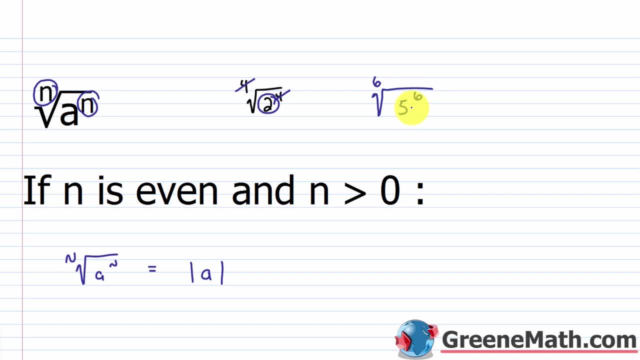 5 to the 6th power is. you can just say, okay, well, if I took 5 and I raise it to the 6th power, whatever number that is, once I take the 6th root of it, I'm going to be right back to 5. so this: 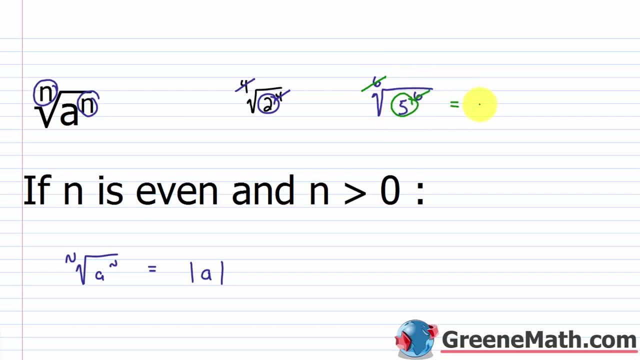 will cancel with this and I'm left with this. so this would be equal to 5. as another example, let's say I was working with a negative and to make it real simple, let's just make it negative 2. so if I had the square root, 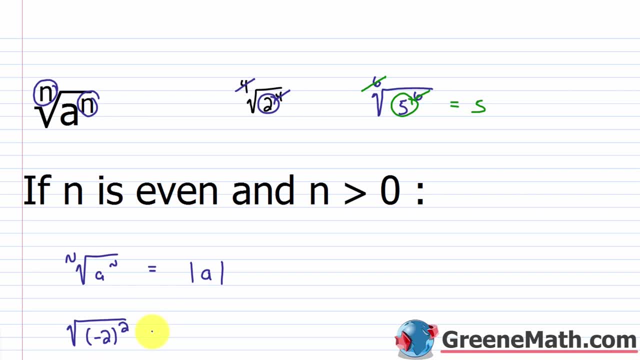 of negative 2 squared, what would that be equal to? well, some of you might say: oh, that's not a real number, you have a negative down there. well, think about squaring this first. if I did negative 2 squared first, that would give me 4. 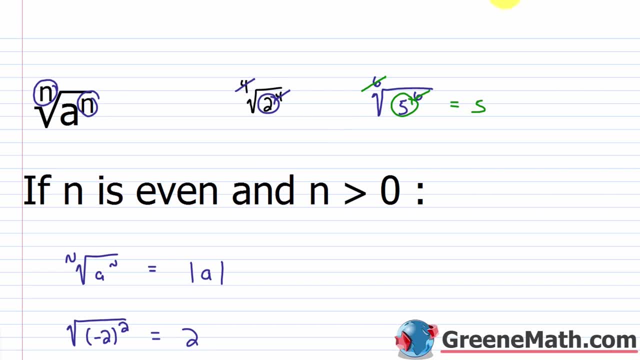 and if I took the square root of 4 I would get 2. so that's where this definition comes into play. notice how we say it's the absolute value of a. so if we're saying a here is negative 2, well, the absolute value of negative 2 is 2. 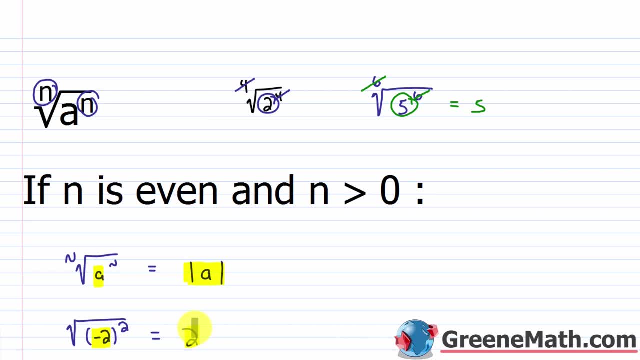 and that comes from that. again, that squaring operation- or in this case it could be anything that's even so- raises them to the 4th power, the 6th power, the 8th power, the 10th power, whatever it is an even number of negatives. 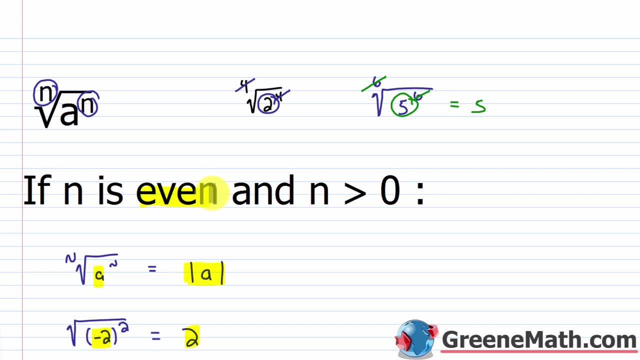 will give us a positive value. then when we perform that root operation, we're going to go back to the absolute value of whatever. that was right, because we took a positive, took the root of it and we went back to whatever the absolute value of that was alright. the next one we want: 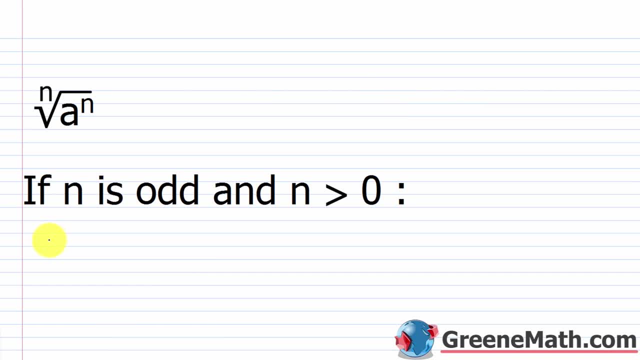 to talk about is the other scenario where n is odd. so if n is odd and n is greater than 0, then what's going to happen in this case? so this is odd and it's greater than 0 in this particular scenario, these two will just cancel each other out. 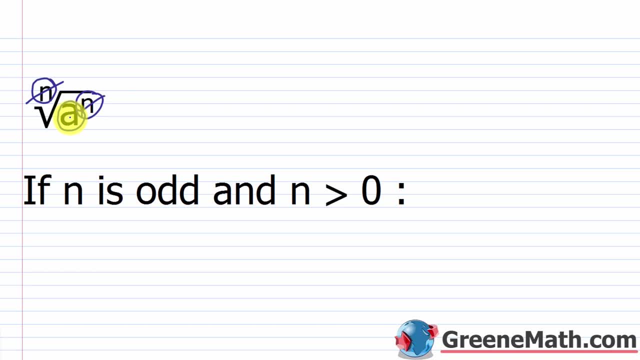 and you're just left with a. so the only difference is, when you have an even involved, you gotta say, in case you're a, in case this radicand was negative, you've got to account for the possibility that you do an even number of factors of that guy right. 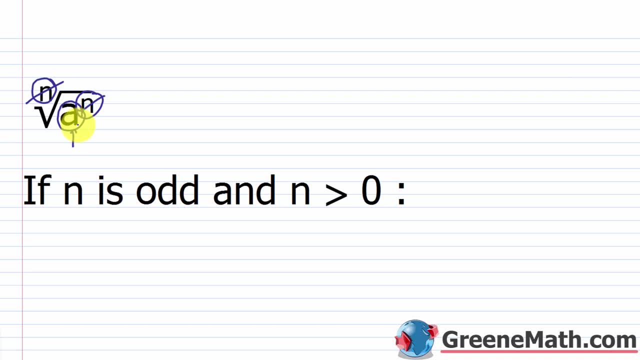 because you're raising it to an even power, it's going to end up being a positive. then you take the root and knocks it back down to the absolute value of that. so that's all we're saying here again, n is even and n is greater than 0. all we're saying is: 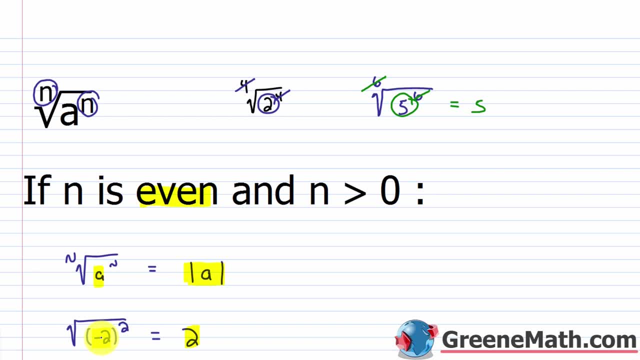 if this guy was negative, an even number of negatives would have made it positive. so you get back to the absolute value of that in this scenario. because n is odd, an odd number of negative factors would give you a negative. it's okay. so as an example, let's say: 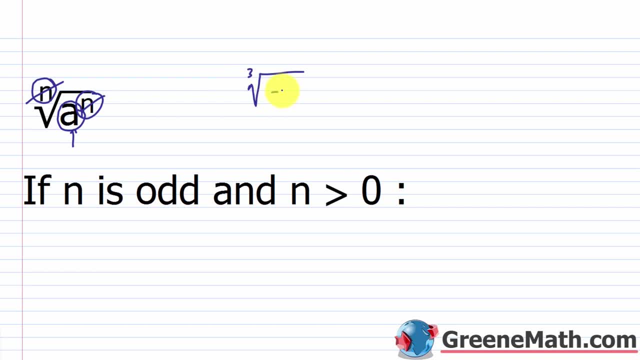 I have the cubed root of, I don't know, negative 2 cubed. well, this is just going to be what this would cancel with this and I just have negative 2. alright, so let's say we saw something like the sixth root of negative 7 to the sixth power. 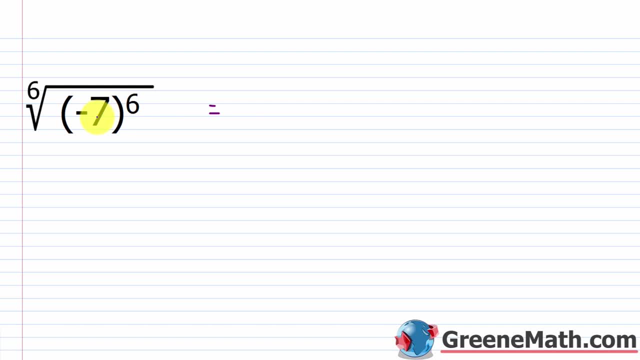 so, again, without even going through and saying okay, well, negative 7 times negative 7, without giving you 6 factors of negative 7 and then taking the sixth root of that, you automatically know that this would cancel with this. but I'm not left with negative 7, I'm left. 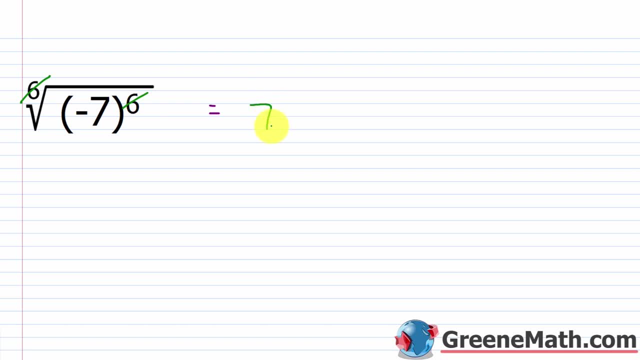 with the absolute value of negative 7, which is 7, right, so it's a little bit more complicated than just cancelling things. I don't want you to make the mistake of just cancelling things and saying, okay, this is negative 7, because that would be wrong. taking negative 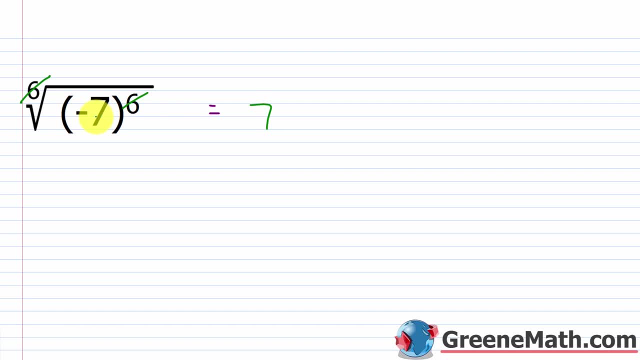 7 to the power of 6 would have made it positive, and then taking the sixth root of that would have brought you back to positive 7. so it's important to realize that this is equal to the absolute value of negative 7, which is 7. 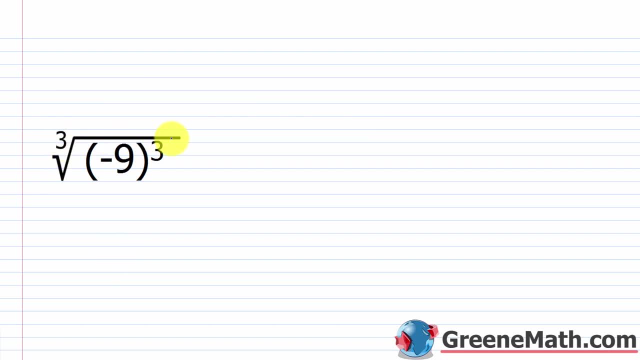 so here's an example where we have an odd index. so we have the cube root of negative 9 cubed. so in this case you can just kind of cancel these and say I'm just left with negative 9. right negative 9 to the third power would still give you a. 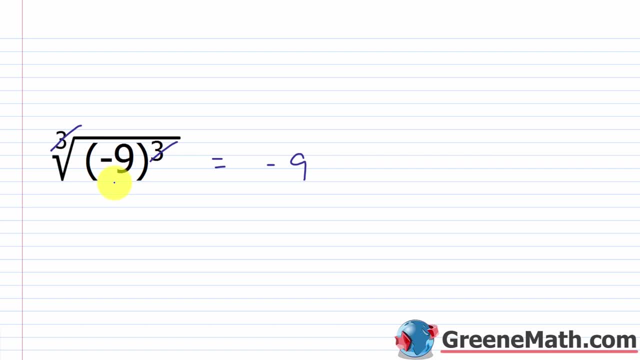 negative result, right. so when I take the cube root of that, it would still be a negative. so when the index is odd, I can just basically cancel these. when the index is even, I want to cancel them, and then I want to use the absolute value here. so 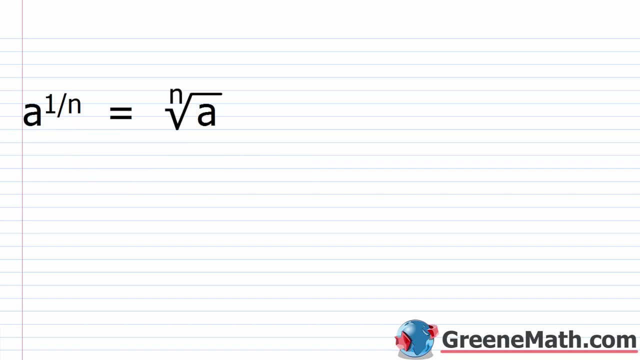 that's the only difference you're watching out for. so now that we've kind of reviewed radicals, let's talk about fractional exponents, or otherwise called rational exponents. so I want you to recall, if you have something like a raised to the power of 1 over n, this is: 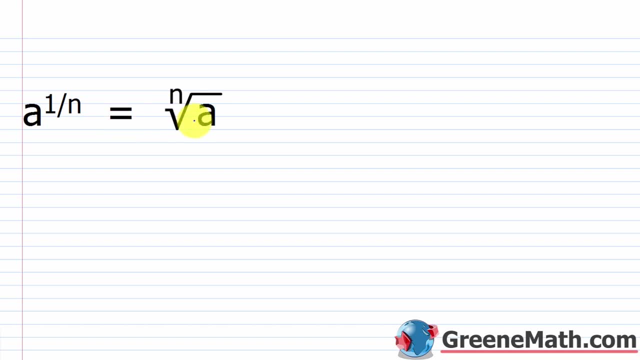 equal to or the same as the nth root of a. so as an example, let's say I had 4 to the power of 1 half. just kind of following this. what would this? be well, this part right here becomes your index. so this part right here would be the index. 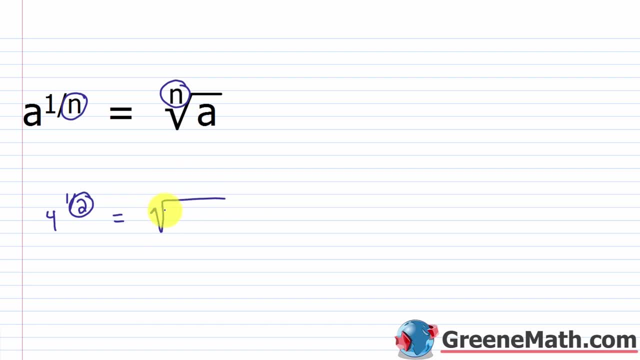 an index of 2 is a square root, so we normally don't display that. but for the purposes here I'm just going to put a 2 here and then 4 just comes over here. so 4 raised to the 1 half power is like: 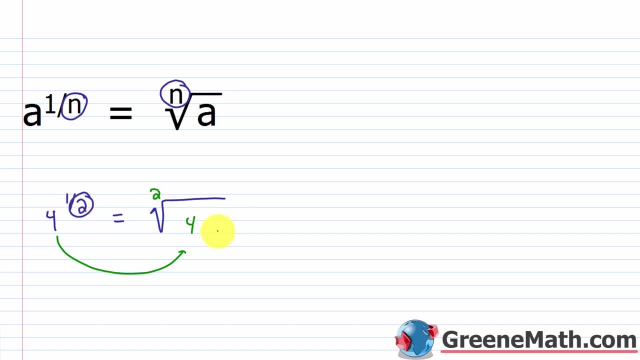 taking the square root of 4, and that should make sense because of the rules for exponents. if I have 4 to the power of 1 half and I multiply it by 4 to the power of 1 half, what would that give me? base stays the same. 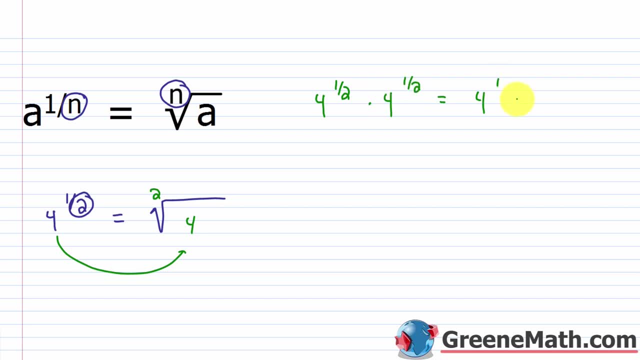 you add your exponents, 1 half plus 1 half is 1, so this is equal to 4. if I did this, using this, and I said: ok, this is the square root of 4 times the square root of 4, we would expect that to be what to be: 4. 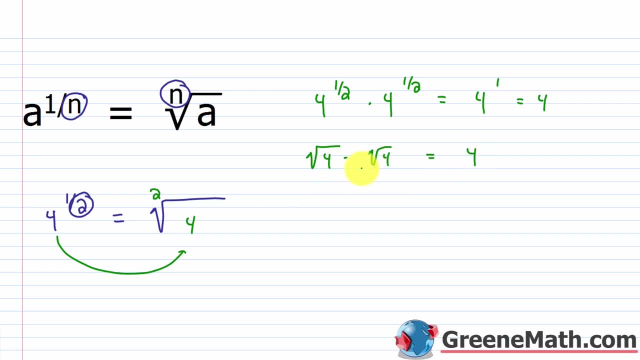 right, the square root of 4 is 2. the square root of 4, again, is 2. 2 times 2 is 4. so it has to make mathematical sense and it does. if I wanted something, let's say as a cube root, ok, a cube root. 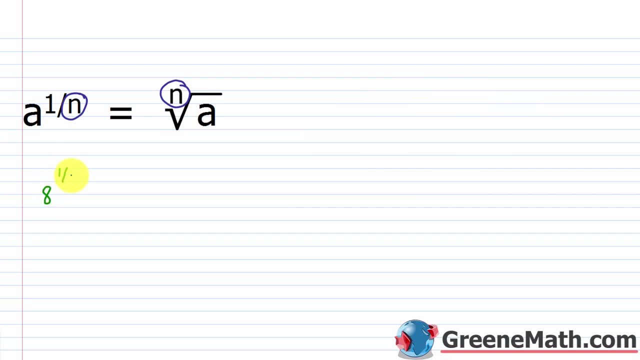 so let's say I had 8 to the power of 1 third. well, this would be the cube root of 8. again, whatever is here in the denominator becomes my index or order, and then it just becomes my radicand. so the cube root of 8 is the same as. 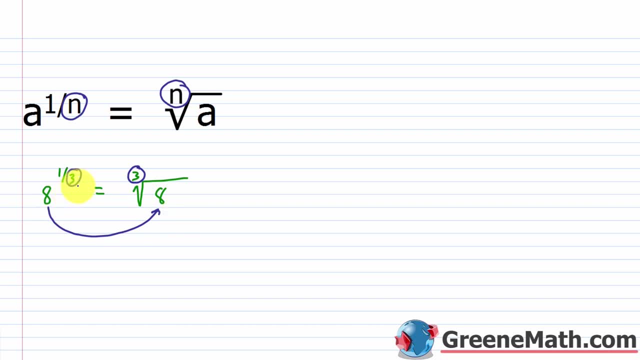 writing 8 to the 1 third power. or you can take something way more advanced. let's say we had I don't know 620, and let's just raise this to the power of 1 eighth as an example. well, this is what. this is the eighth root. 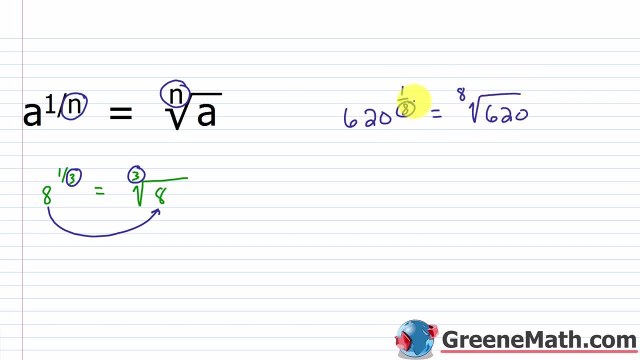 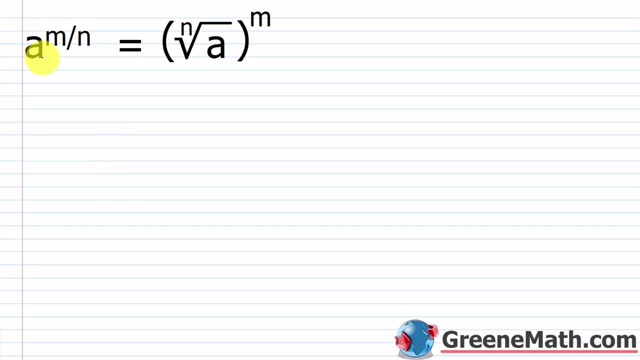 of 620, because this part right here goes here and this part right here goes here. so the other thing we need to know: with this, let's say we have a raised to the power of m over n. this just gets split up into the nth root of a and this is: 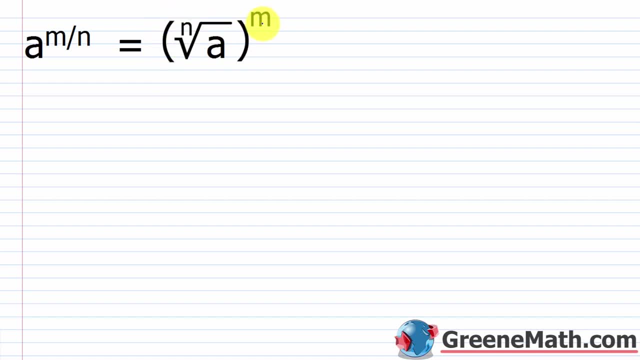 raised to the power of m. so a good example of this would be something like 9 to the power of, let's say, 3 halves. so, just following this, what would you see? again, the denominator becomes the index, this becomes the radicand, and then this: right here we're going to raise everything to. 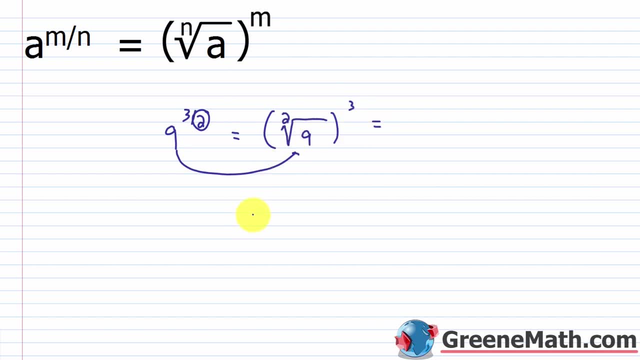 that power. so if I took the square root of 9, I would get what? I would get 3, and then if I cubed 3, I get what. 3 times 3 is 9. 9 times 3 is 27. now there's other ways to do that you. 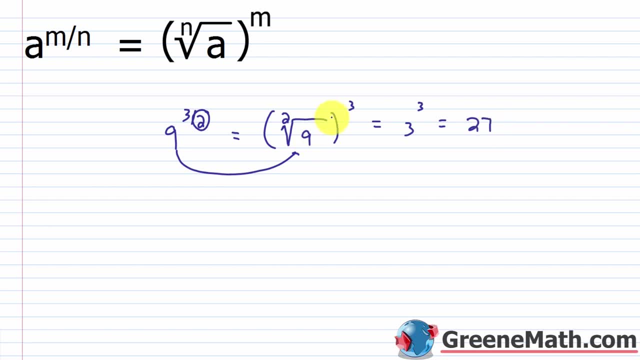 might see your book tell you to take this guy and raise it to the third power first. so I could also say that 9 to the 3 halves power is what it's, 9 cubed. okay. so 9 is raised to that power and then we take the. 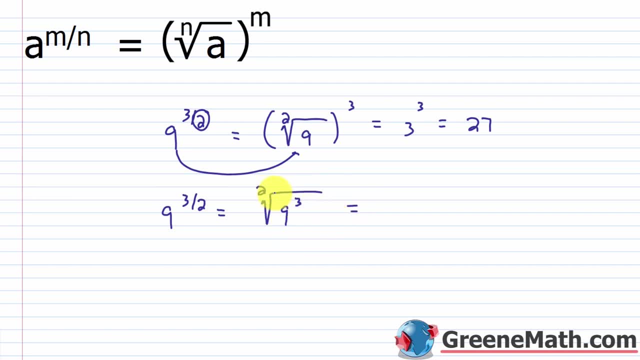 square root of that, but this produces a bigger number to take a square root of, and so it's not usually what you want to do. 9 cubed is 729, so it would be the square root of 729 which is going to give you 27. alright, so let's just 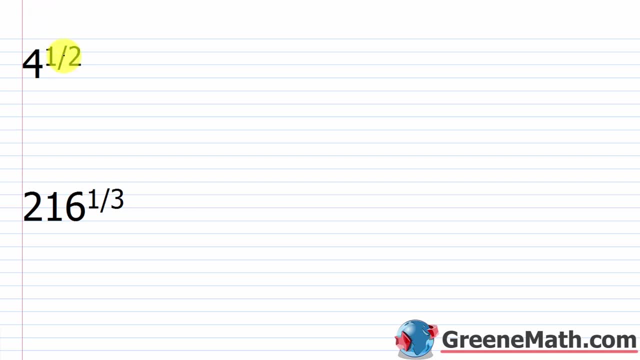 look at some examples. we have 4 to the power of 1 half. we know that's just 1. if you raise something to the power of 1 half, you're just asking for the square root. so it's the square root of 4. now again you take this: 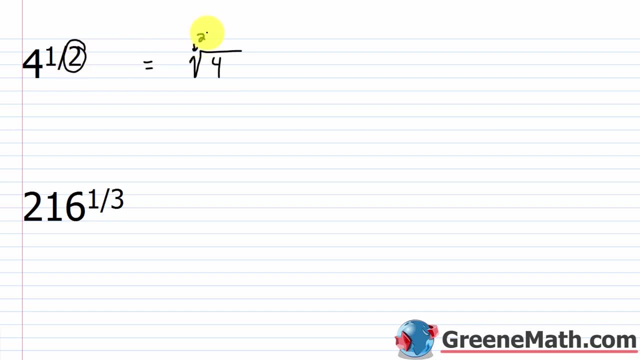 right here, that's in the denominator, that's your index. so the index would be a 2 on a square root. we just don't show that this right here. this 4, that number, that's the base when we're talking about an exponent, becomes the radicand. so you basically: 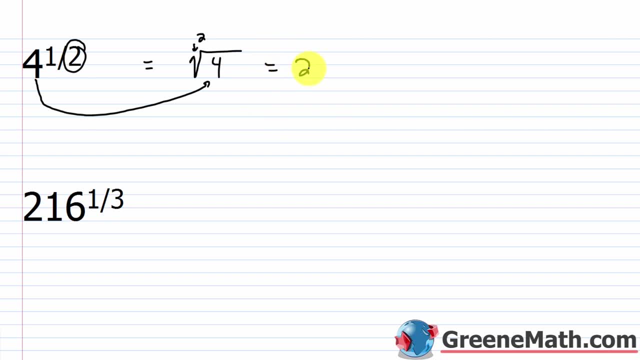 get the square root, or the principal square root of 4, which is 2, if you look at 216 to the power of 1. third, we're asking for the cube root of 216 again. this denominator here becomes the index, 216 becomes the radicand. 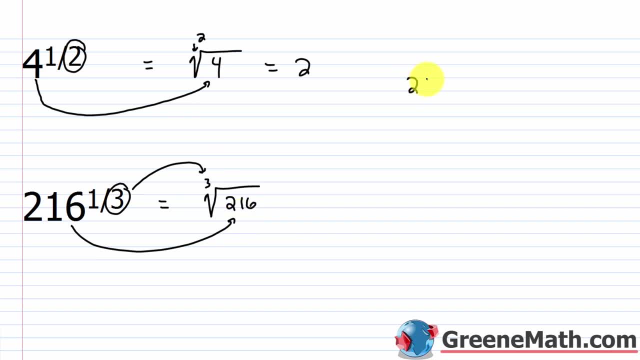 so what is the cube root of 216? so if you don't know that off the top of your head, just look at the last two digits. it's a 16. so you know. this is divisible by 4, so this would be 54 times 4, 4 is, of course, 2 times. 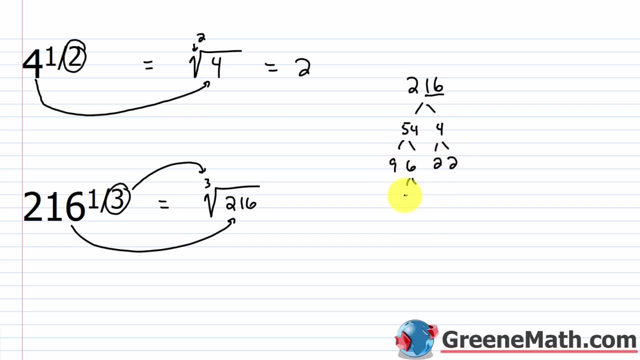 2, 54 is 9 times 6, 6 is 3 times 2, 9 is 3 times 3. now, what do I have here? I have 1, 2, 3 factors of 3 and 1, 2, 3 factors. 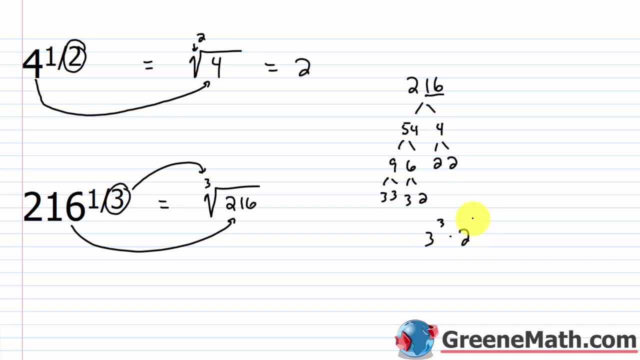 of 2, so we've got 3 cubed times 2 cubed. basically, 3 times 2 is 6, so it's 6 cubed. so this is equal to what? it's equal to 6, because 6 cubed would give me. 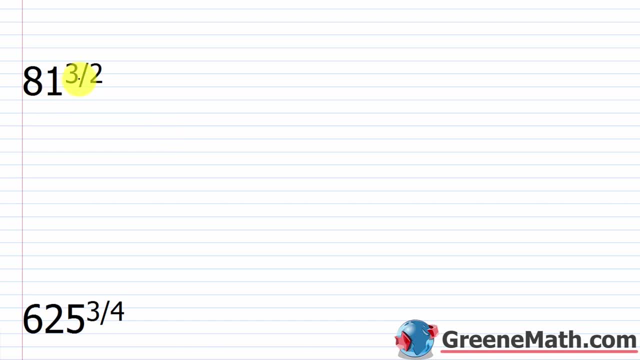 216. so let's take a look at a harder example. so we have 81 to the power of 3 halves. 81 is going to be my radicand. my index is going to be what it's going to be a 2. it's always the denominator. 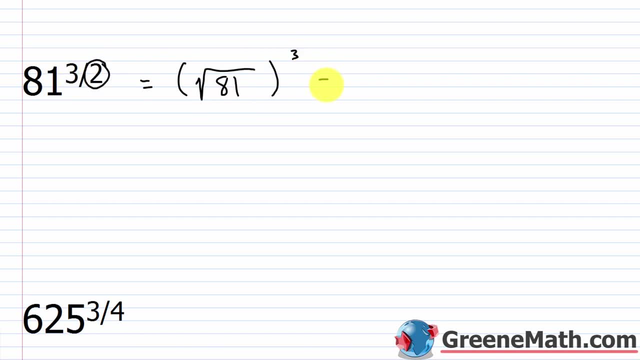 and then I'm raising this whole thing to the power of 3. so the square root of 81 is 9. 9 cubed, as we just found out, was 729. alright, let's take a look at 625 to the power of 3. fourths: 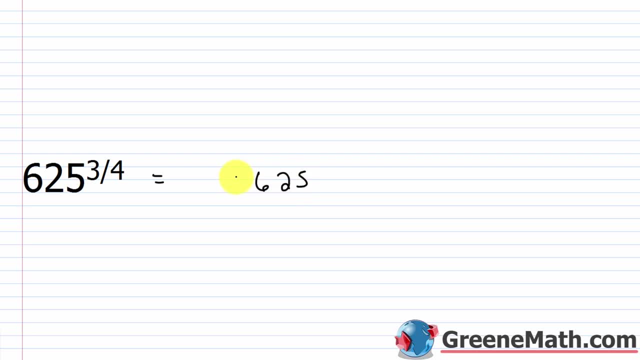 so again, 625 is my radicand and the index. here is what it's, a 4. and then we want this all raised to the third power. so what is the fourth root of 625? most of you know that is 5. 5 times 5 is 25. 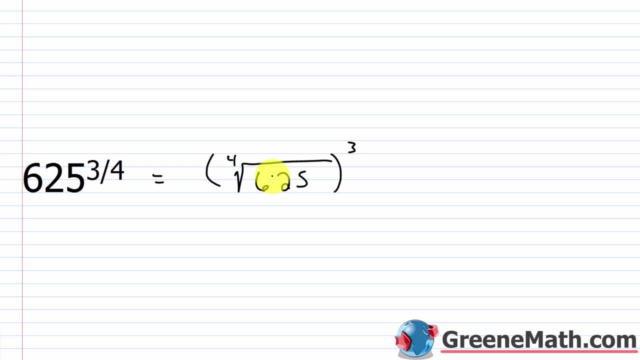 25 times 5 is 125. 125 times 5 is 625. so if this becomes 5, when I cube that, I go back to what. I go back to 125. what about if we mix some things up and we ask for 16? to the power of. 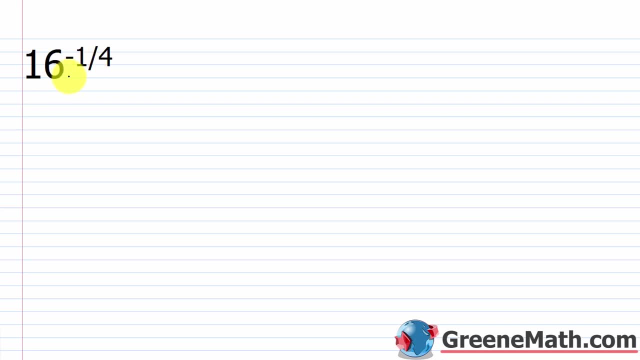 negative 1. fourth. so what am I asking for here? well, again, I want the fourth root, I want the fourth root of 16, and then I would raise everything here to the power of negative 1, so I can go ahead and take this first. well, this is 2, so this would be 2. 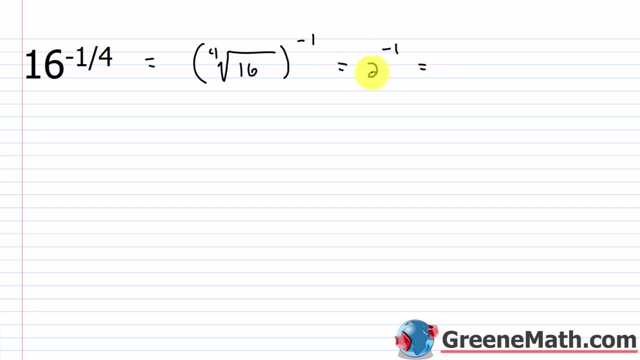 to the power of negative 1, which is what it's just. take the reciprocal of the base, so 1 over 2. raise this to a positive 1, which is basically just 1 half. now the other way to do this. if you wanted to, you could say: 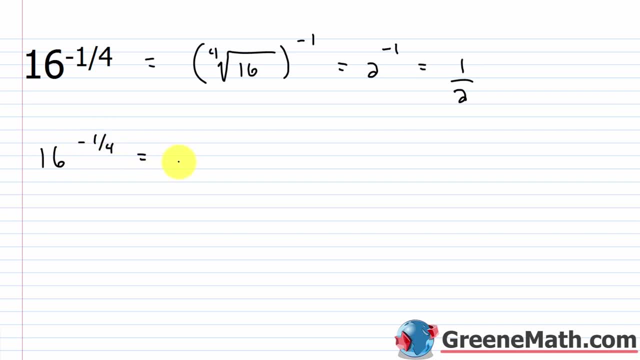 ok, I have 16 to the power of negative 1. fourth, well, you could have started out by saying: I have 16 raised to the power of negative 1, and then I'm going to take the fourth root of that same answer. either way, this would. 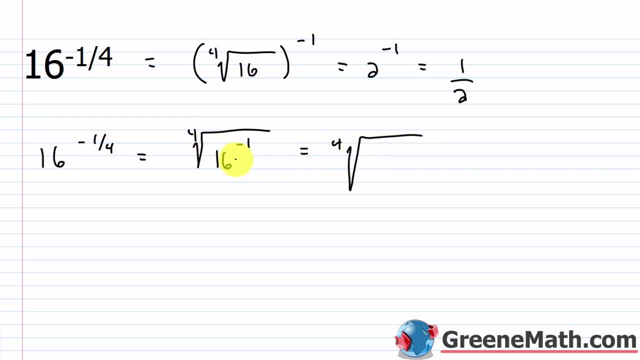 be what this would be the fourth root of take the reciprocal of this. this is 1 over 16, and it's a little bit more complex here because it's a fraction, but just think about the fourth root of 1 over 16. well, 1 half times, 1 half times. 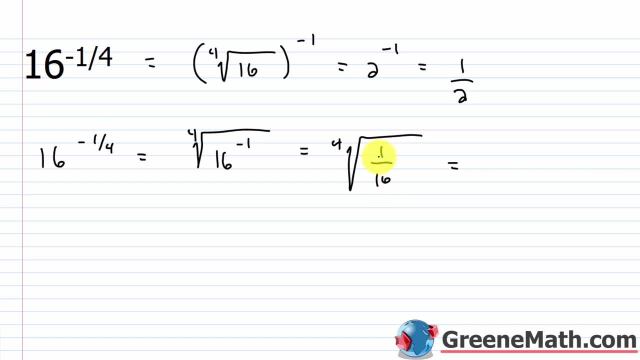 1 half times 1 half is going to give you 1, 16. you know, 1 to the fourth power is 1, so that's easy. and then what to the fourth power, 16? well, that's 2, so you end up with 1 half. 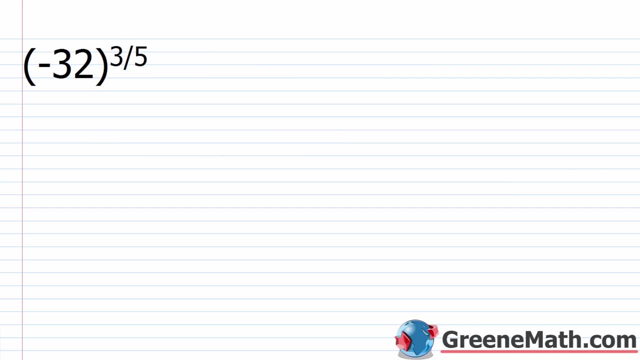 either way. now, what about something like negative 32 to the 3 fifths power? well, again we're looking at, we have negative 32, and then I'm going to take the fifth root of that and I'm going to raise the whole thing to the third power. 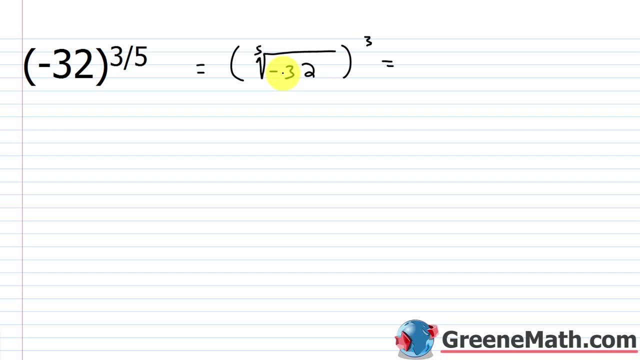 so what's the fifth root of negative 32? that's going to give us negative 2 and we want to cube that negative 2. cubed is negative 8. but the next one we're going to look at 5 raised to the power of 5 thirds. 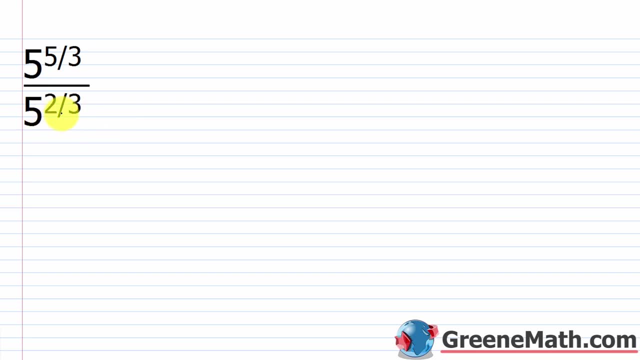 over 5, raised to the power of 2 thirds. now, just as we saw when we worked with exponents in the past, if you have the same base which we have- a base of 5, a base of 5- and you're dividing, you subtract the exponent in the numerator. 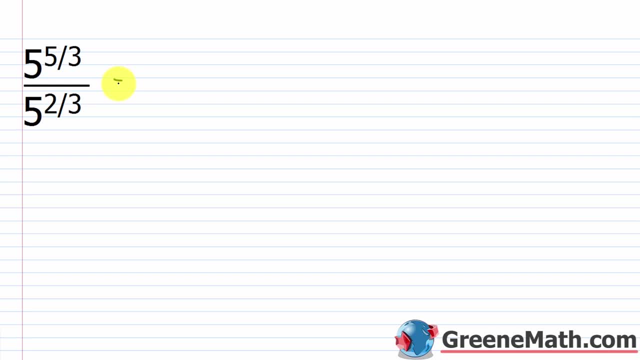 minus the exponent in the denominator. so 5 just stays the same and we would do 5 thirds minus 2 thirds. same rules apply. no matter what you're working on, no matter how complex it is, you always go back to those basic rules that you learned. 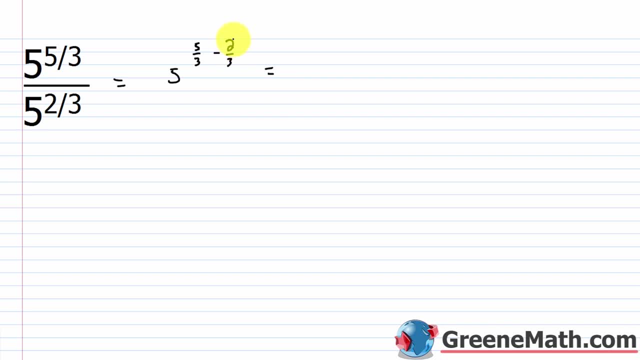 so 5 minus 2 is what that's 3. so you would have 5 raised to the power of 3 over 3, which is 5 to the power of 1. it's just 5. let's say: we take a look at m squared. 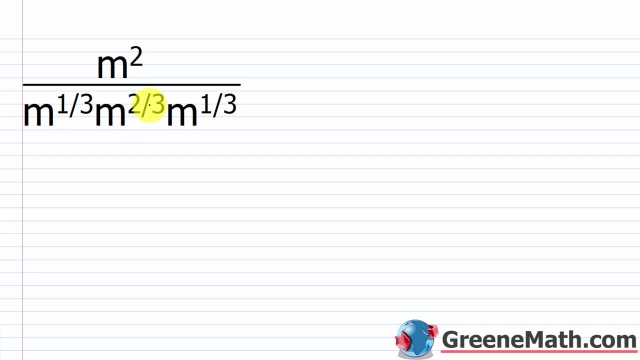 over m to the power of 1 third times m to the power of 2 thirds times m to the power of 1 third. so again, same rules apply. so m squared over. I'm just going to use my product rule for exponents. m would stay the same. 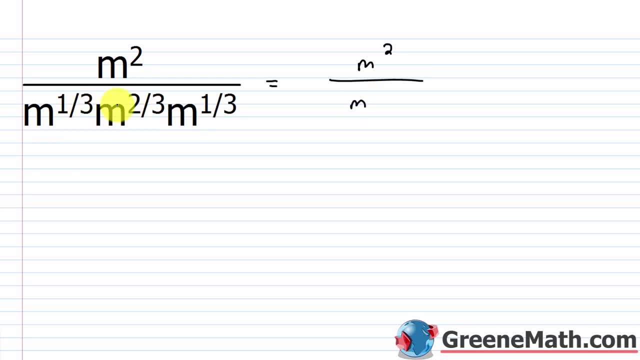 and we would add all these exponents. so we know that 1 third plus 2 thirds is 3 thirds. 3 thirds plus 1 third is 4 thirds. so what would happen here is, if I'm dividing, m stays the same and we would do 2. 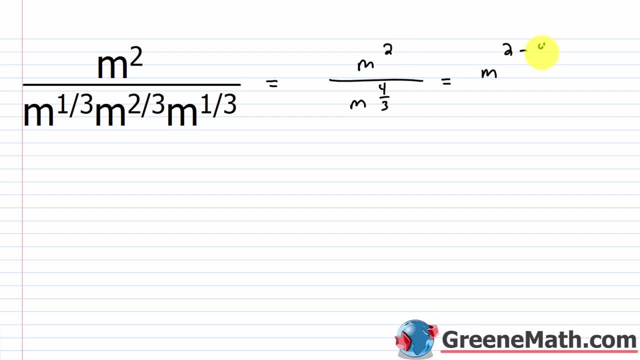 which is the exponent in the numerator, minus 4 thirds, which is the exponent in the denominator. to get a common denominator, I would write 2 as what 6 thirds, and we'd end up with m to the power of 6 minus 4 is 2 and then over. 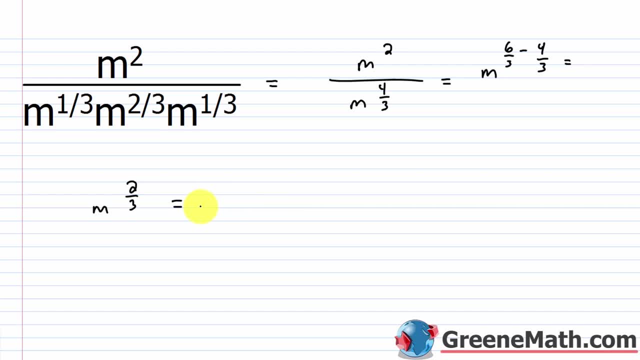 3, so you can leave it in this format. or you could write that you have the cube root of m, that's squared, or you could say you have m squared and take the cube root of that. all of these are the same. what about m? cubed squared times, m? 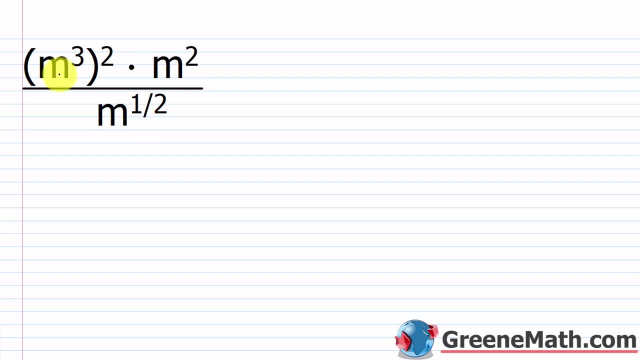 squared over m to the power of 1 half. well, using my power to power rule here, I know this would be m to the 6th power and times m squared. all I would do is add exponents here, so m would stay the same. 6 plus 2 is 8, so this would basically. 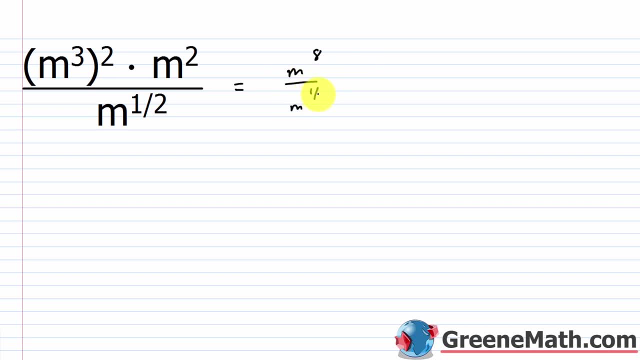 be m to the 8th, power over m to the power of 1 half. so m stays the same and I would take 8 and I would subtract away a half. so let's write this as 16 over 2, minus 1 over 2, this would equal. 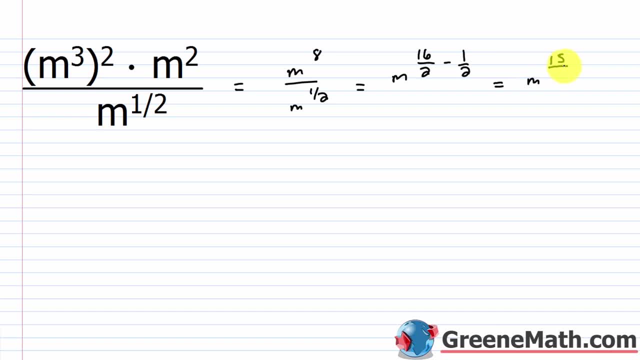 m to the power of 15 over 2. again, you could leave it like that: or you could write that you have the square root of m raised to the 15th power, or you could say you have m to the 15th power and then you could take the square root of that. 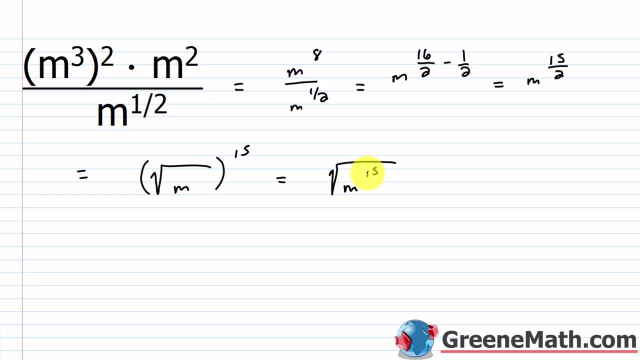 right, all of these, this one, this one and this one mean the exact same thing. alright, for the last one. we have x squared raised to the 2, 3rd power times, x to the power of 1 half over, x to the power of negative 3 halves. 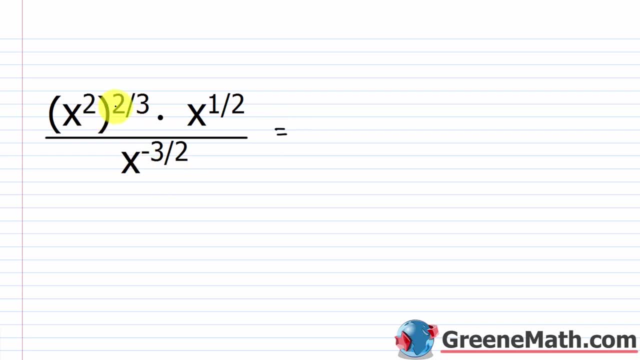 so if I look at this, I use my power to power rule. I would multiply 2 times 2 and get 4, so this would be x to the power of 4 3rds, and then we multiply by x to the power of 1 half and 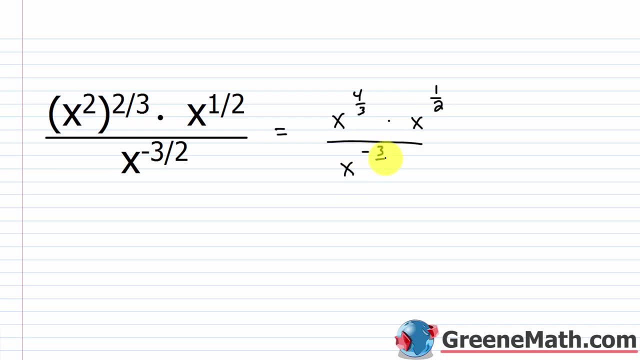 of course this is over x to the power of negative 3 halves. so let's put this as equal to. let's deal with the numerator first. so we have what we have, x staying the same, and we're going to add the exponent. so if I add 4 3rds, 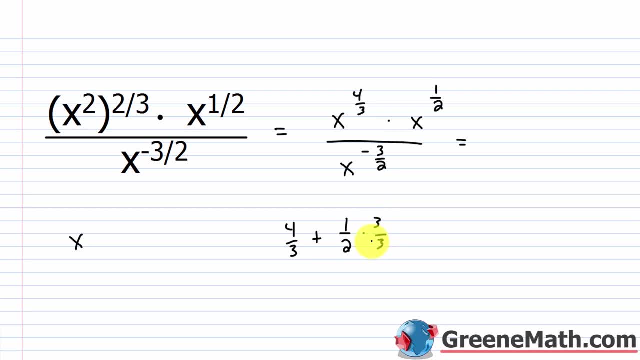 plus 1 half. multiply this by 3 over 3. multiply this by 2 over 2. 2 times 4 is 8, so you would have what you'd have: 8 over 6 plus 1 over 3 is 3 over 6. 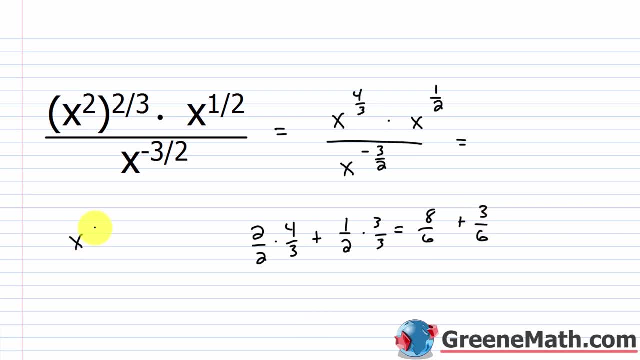 8 plus 3 is 11. so this would be x to the power of 11 sixths. then this is over x to the power of negative 3 halves. now I don't need to do anything fancy here, other than leave x the same and then just. 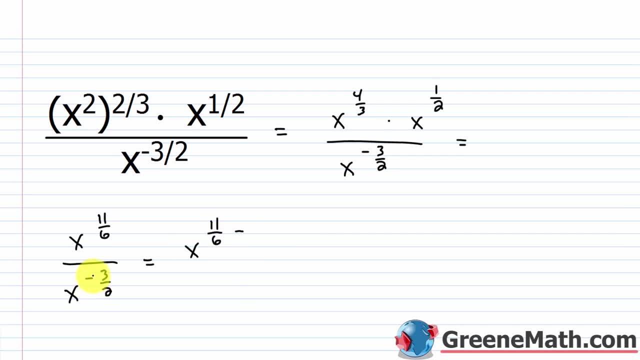 subtract, so I would do 11 sixths minus a negative. notice that that's a negative and I'm subtracting it away. so that's plus a positive 3 halves. so to get a common denominator, let's multiply this by 3 over 3 and this would be 9 sixths. 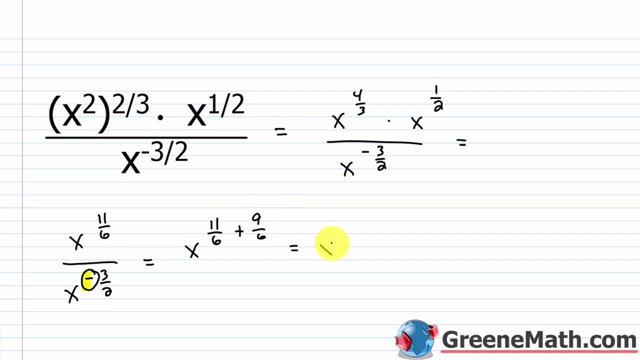 9 sixths. so this would be x to the power of 11 plus 9 is 20 over 6. now, if you get a scenario like this, you can reduce this. we know that 20 and 6 are each divisible by 2, so we can really. 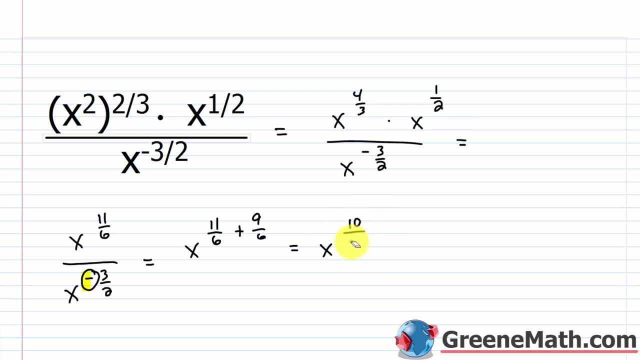 say this is 10 over 3. and then what we want to do is say, okay, we have the cube root of x and this is raised to what, the 10th power. or again you could also say: you have x to the 10th power. 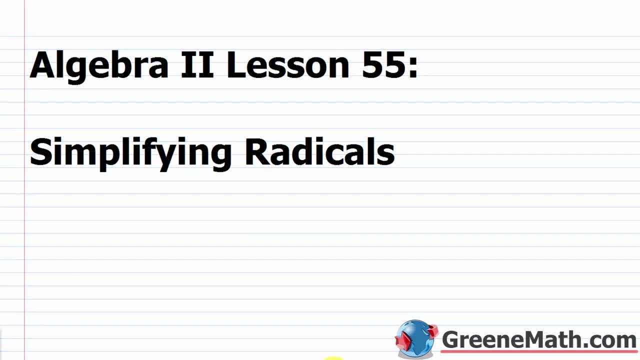 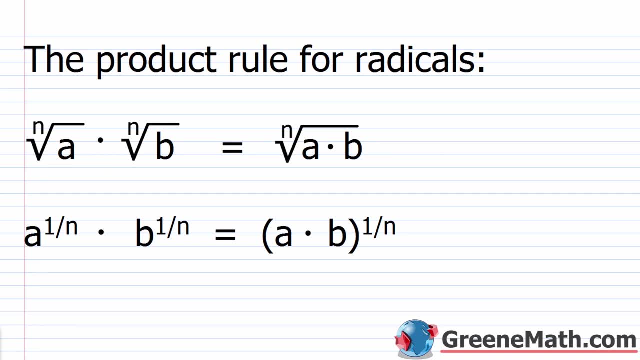 and you're taking the cube root of that. hello and welcome to algebra 2, lesson 55. in this video we're going to learn about simplifying radicals. so again we have another lesson where we're just kind of covering or refreshing our memory on things that we learned back in algebra 1. 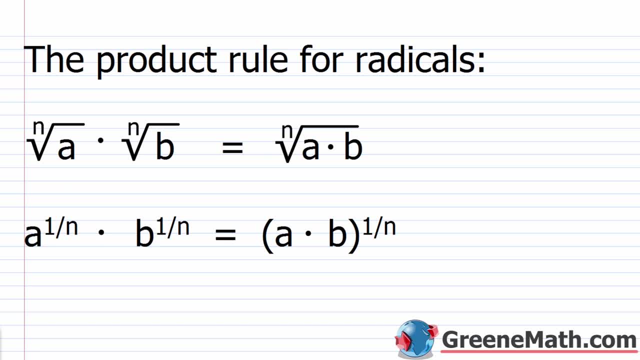 so I want to start by talking about the product rule for radicals and the quotient rule for radicals before we get into actually how to simplify a radical. so the first thing, again, the product rule for radicals. if we see something like the nth root of a times the nth root of b, we could 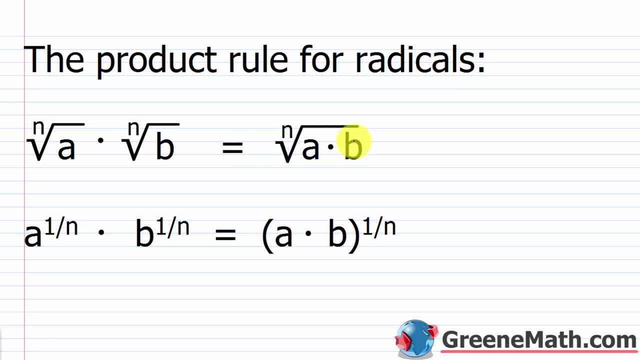 say: this is equal to the nth root of a times b. now when we look at again very generic things like this, things we'd see in our textbook, a lot of you get confused and say: what does that really mean? we're saying, if the index is the same, 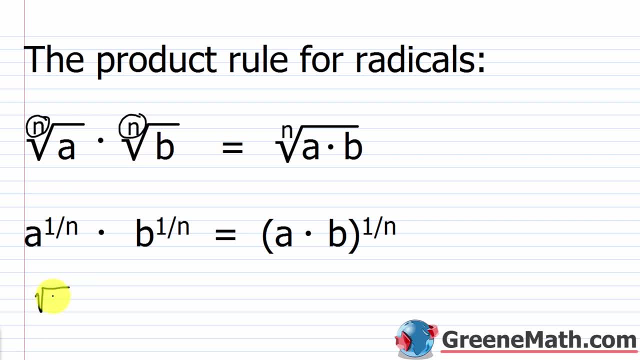 so, in other words, if I had something like the square root of 2 times the square root of 3, so the index here is a 2, the index here is also a 2, this is going to be equal to the square root of. in this case, you have a. in this case, you have. 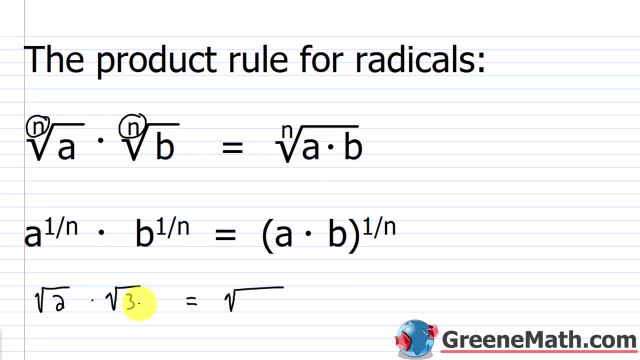 b. so we combine them and say a times b. in this case we have 2, in this case we have 3. so we combine them and say 2 times 3. so this is the square root of 6. that's all. it is okay in. 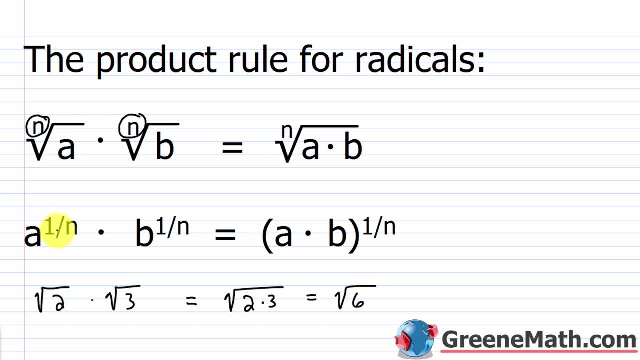 exponent form. remember, if we raise something to the power of 1 over n, it's the same thing as taking the nth root of it. so the nth root of a can be written as a to the power of 1 over n and the nth root of b can be written as b to the power of 1 over. 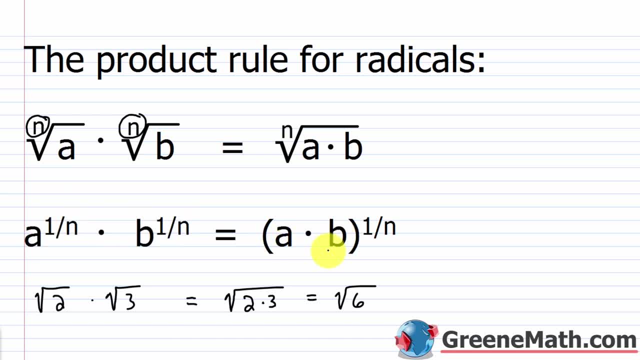 n, so you multiply the two together and we're just showing this with exponents. it's the same thing between here and here. we have a times b inside a parenthesis and it's raised to the power of 1 over n. so as an example here I could say this is 2 to the power of. 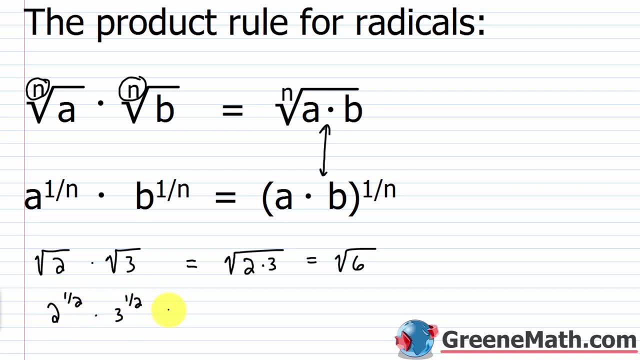 1 half times 3 to the power of 1 half. this would be equal to 2 times 3 to the power of 1 half, or 6 to the power of 1 half, which again we know is the square root of 6. 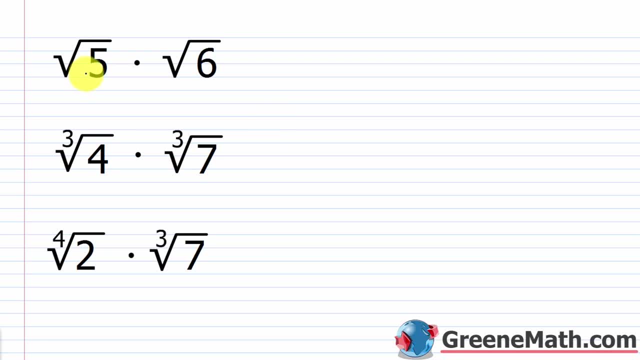 alright, let's take a look at some examples. let's say we have the square root of 5 multiplied by the square root of 6. we can combine these two and just say it's the square root of 5 times 6, which is the square root of. 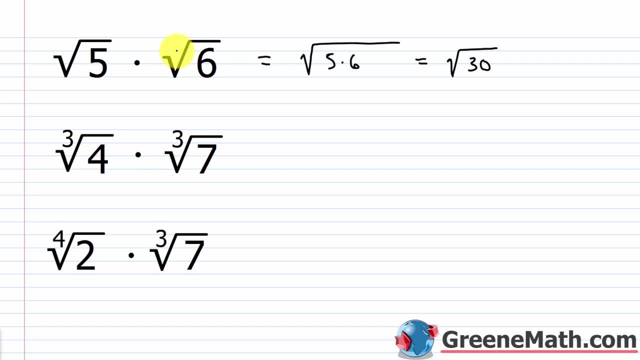 30 and again notice how your index here is a 2, your index here is a 2, so same index. so we're allowed to combine them in that way. for the next one, we have the cube root of 4 multiplied by the cube root of 7, so same index. 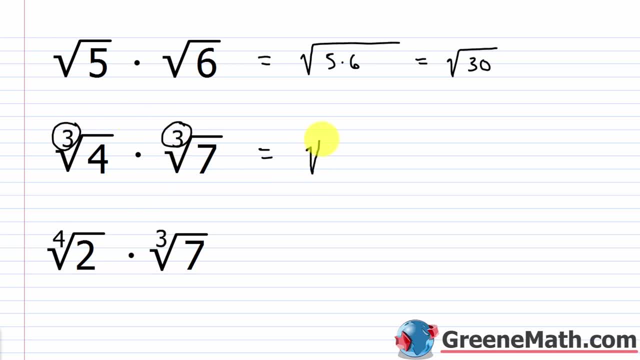 you got a 3 here and a 3 here, so that would be the cube root of 4 times 7, which is 28. now for this one, I gave you an example where you can't use this method. you have the fourth root of 2 multiplied by the. 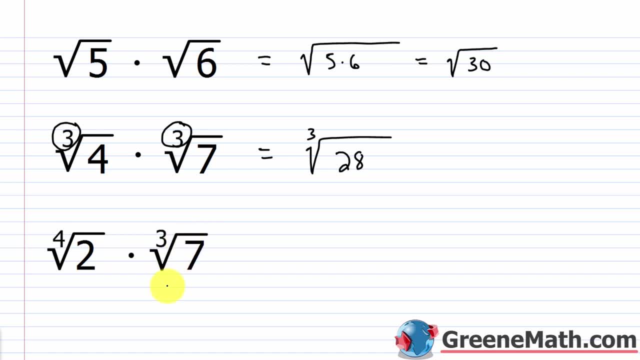 cube root of 7. now there is a way to combine this and we'll get to that at the end of the lesson, but you can't do it using the product rule for radicals. to use the method that we've been doing, you've got to have the same index. 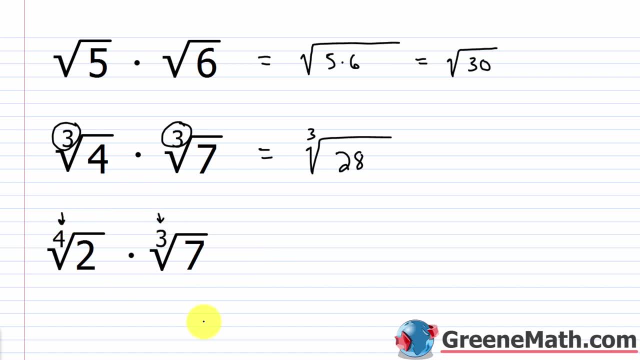 again, this is a 4 and this is a 3, so you're not going to be able to combine those using this method. alright, here's an example with some variables involved. so suppose we had the 7th root of 20x cubed multiplied by the 7th root. 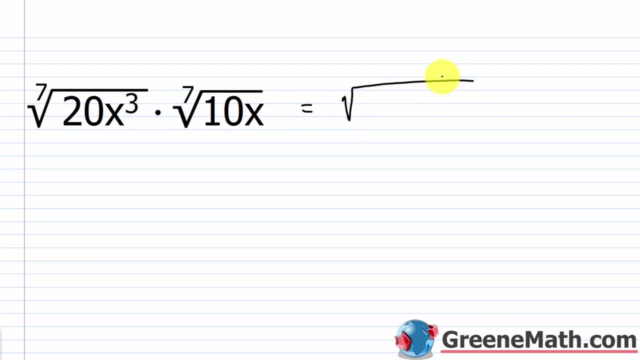 of 10x, so it would be the 7th root of what. 20 times 10 is what, that's 200, and then x cubed times x is x to the power of 3 plus 1, which is 4, so you'd have the 7th root of. 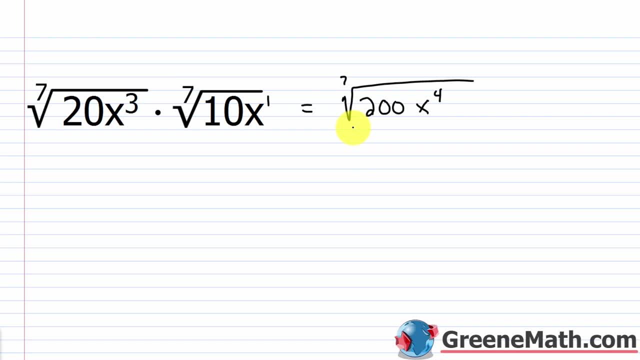 200x to the 4th power. so you get the idea again. we talked about this back in algebra 1. even if you didn't see it in algebra 1, it's very, very simple: if the indexes are the same and you're multiplying, just set up that root. 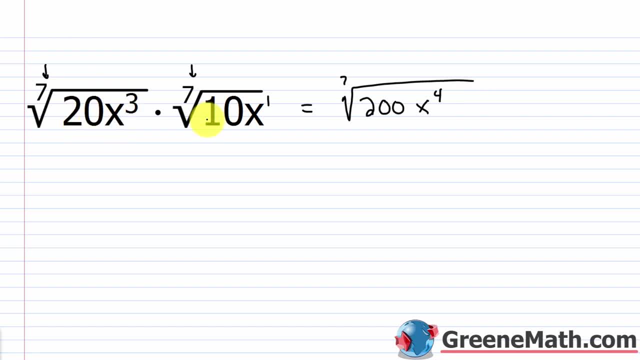 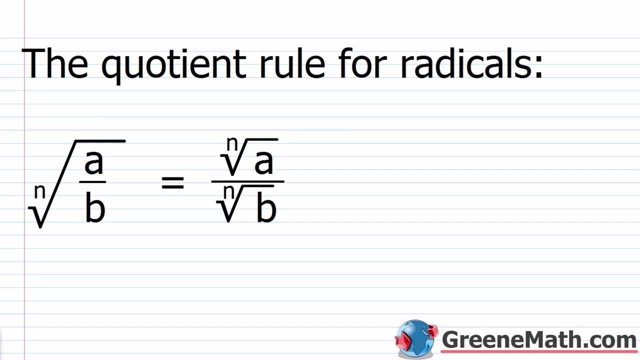 with that same index and just multiply the two radicands together, and that's all we're doing. alright, now let's talk about the quotient rule for radicals, which is pretty much very similar. if you have the nth root of a over b, you can say: this is equal to the nth root of a. 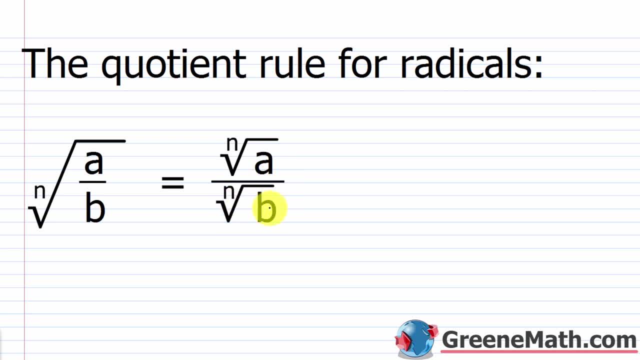 divided by or over the nth root of b, so it just allows us to split things. so, in other words, if I had the square root of, let's say, 1- 4th, I could split this up into the square root of 1 over the square root of 4. 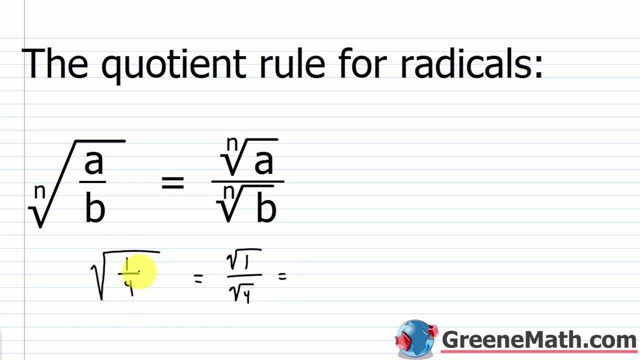 and then it's a lot easier to figure this out. instead of looking at a 4th and saying, well, what number times itself would give me a 4th, I could say: what number times itself would give me 1, that's 1, what number times itself would give me 4. 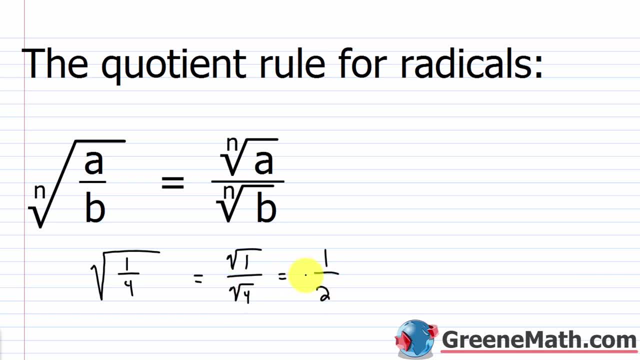 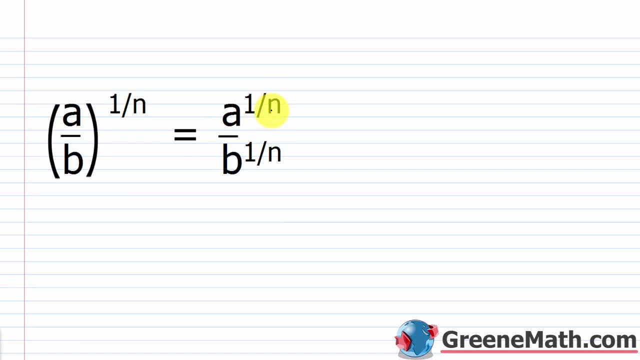 that's 2, so this ends up giving me 1 half. so we can also show this in exponent form. we have a over b raised to the power of 1 over n. we just say this is equal to a raised to the power of 1 over n. 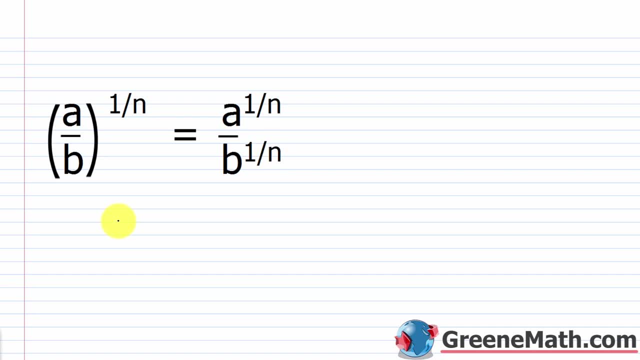 over b, raised to the power of 1 over n. it's no different than if I had something like, let's say, 10 over 2 and this is squared. this is the same as 10 squared over 2 squared. either way, if I do 10 over 2, 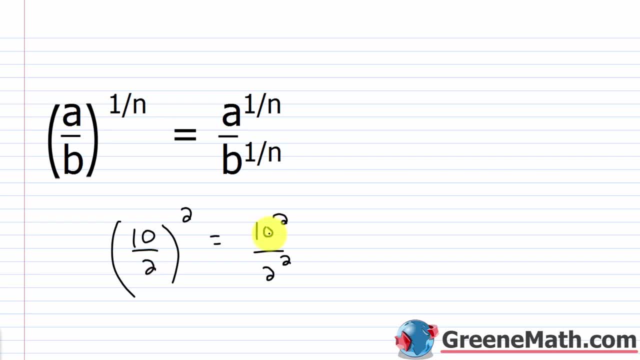 that's 5,. 5 squared is 25. if I do it this way, 10 squared is 100, 2 squared is 4, 100 divided by 4 is also 25. so same result either way. so let's look at a few examples of this. 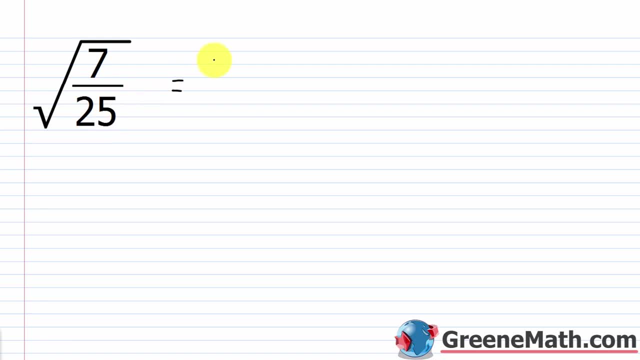 we have the square root of 7- 25ths, so all we're going to do is break this up. we have the square root of 7 over the square root of 25. now, 7 is not a perfect square, so I'm going to leave that as just the square root of 7. 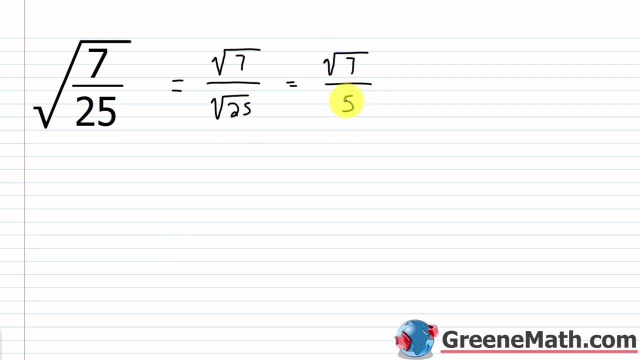 and then the square root of 25 is 5, so we'd end up with the square root of 7 over 5. now we have the cube root of 8 over 216, so I'm going to break this up into the cube root of 8. 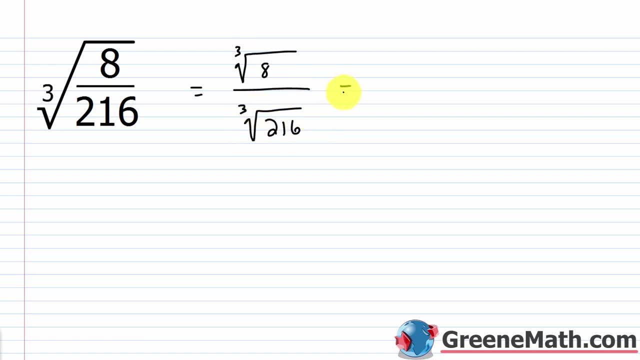 over the cube root of 216. the cube root of 8 is 2, the cube root of 216 is 6 and we can reduce this fraction. don't stop and say, oh well, I have to finish there. it's the same rules that apply throughout all of. 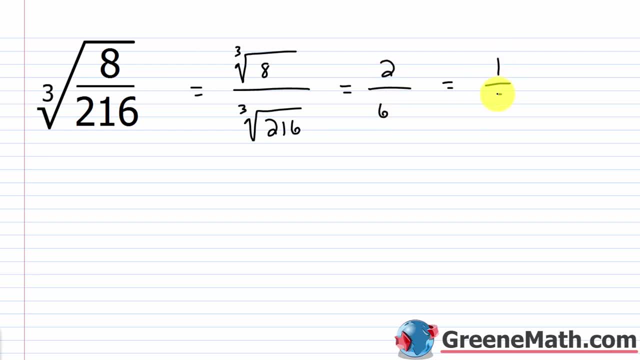 mathematics, if you have 2 over 6, that's the same as 1. third, cancel a common factor of 2. alright, then what about the 5th root of negative 1 over 32? so this would be the 5th root of negative 1. 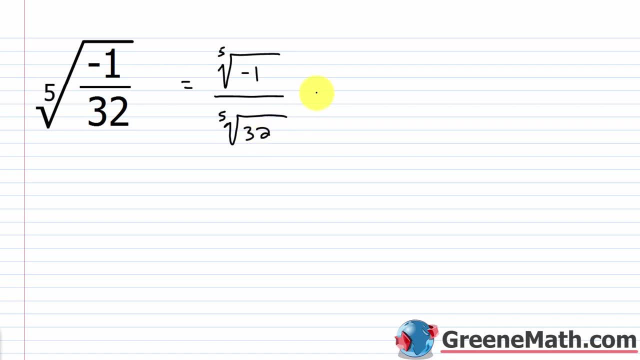 over the 5th root of 32. so the 5th root of negative 1 is just negative 1, because negative 1 times itself 5 times would give me negative 1 one back and this is over the 5th root of 32. 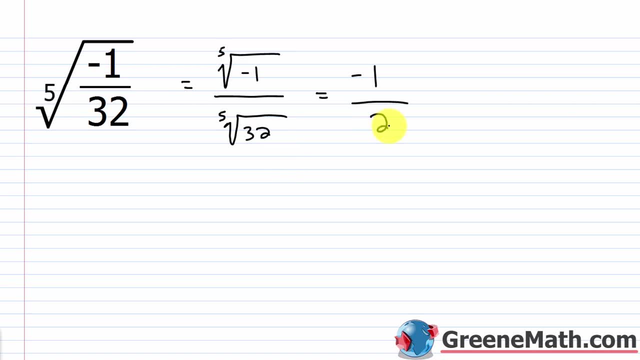 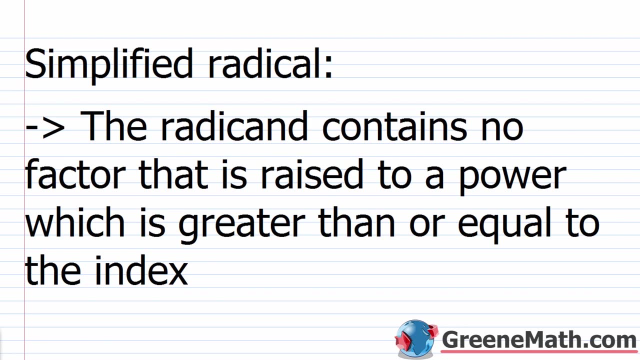 is 2, so this is negative 1 half as the answer. alright, so now let's talk about what we came here for, which is how to simplify a radical, and again it's something you need to do to get full credit on your answer. it's just kind of like when you reported fractions. 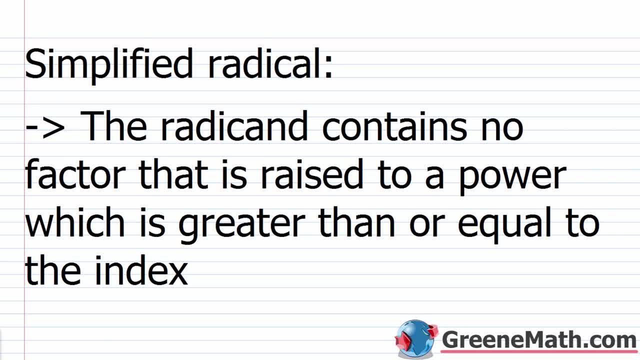 but you didn't simplify them and your teacher would take points off. you need to follow these rules because this is what's expected of you. so, in a simplified radical, the first and the most important thing is that the radicand contains no factor that is raised to a power. 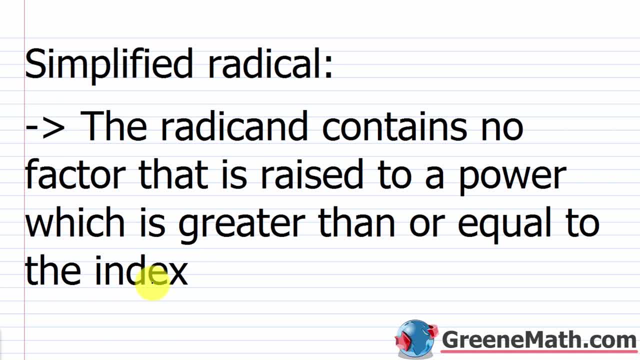 which is greater than or equal to the index. now, that might seem kind of challenging if you just read it, but really it's quite simple. if I had something like the square root of 20, for example, if you think about factors of 20, there's a perfect square inside of there. 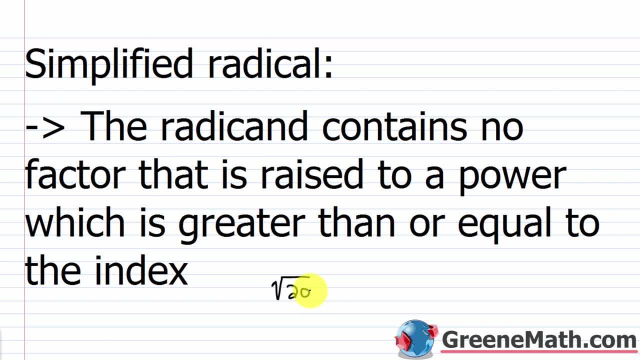 so all we're saying is that it would be simpler if I rewrote this and said: hey, 20 is really 4 times 5, or 2 times 2 times 5, so 4 is a perfect square. so I could write this as the square root of 4. 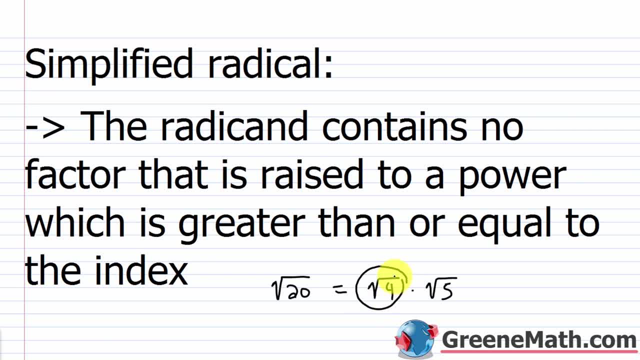 times the square root of 5, and you'd say: well, hey, this square root of 4, that's really just 2. so now I could further simplify this and say: this is 2 times the square root of 5. so all we're saying is that this is preferred. 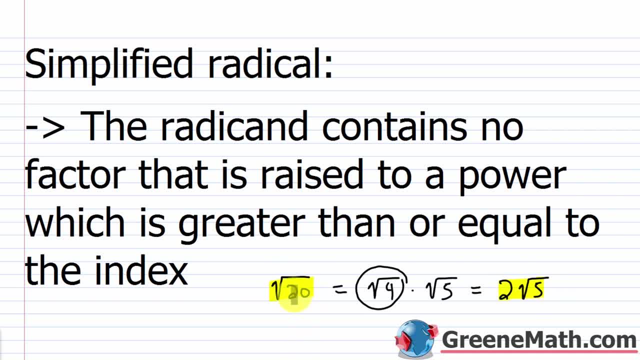 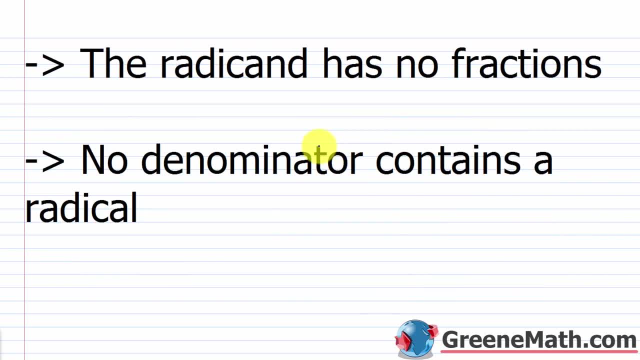 to this because we're taking out the perfect square, which was 4, into a factor of 20 and we wrote the square root of 4 as 2, alright, so the next one is a little confusing. we say the radicand has no fractions, so this ties into. 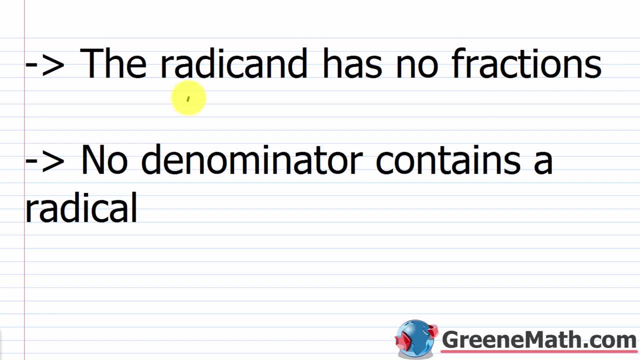 your quotient rule for radicals. so let's say, you saw something like the square root of 5 over 36. so this radicand contains a fraction. it also has 36 involved. 36 is a perfect square. so it's kind of two things you want to take care of. 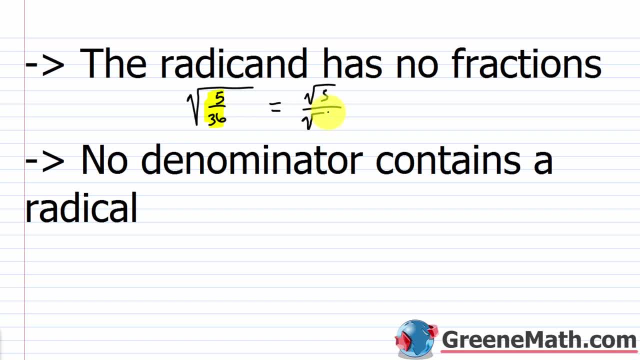 so for this you would split it up into 5 over the square root of 36, so this would end up being the square root of 5- and 5 is not a perfect square, so we can't do anything with that- and the square root of 36 is just 6. 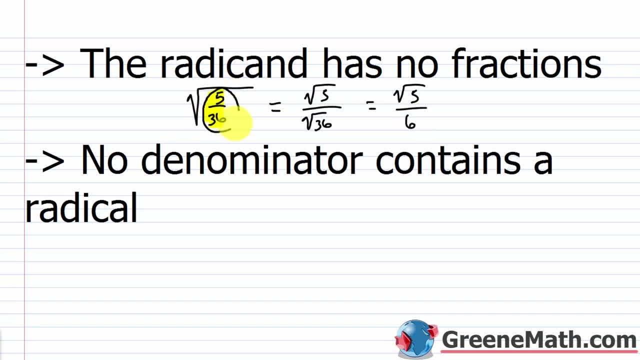 so now we started with something that had a fraction in the radicand. we just have the square root of 5 over 6, and my radicand here of 5 does not contain a fraction. alright, so the next one- we have no denominator- contains a radical. 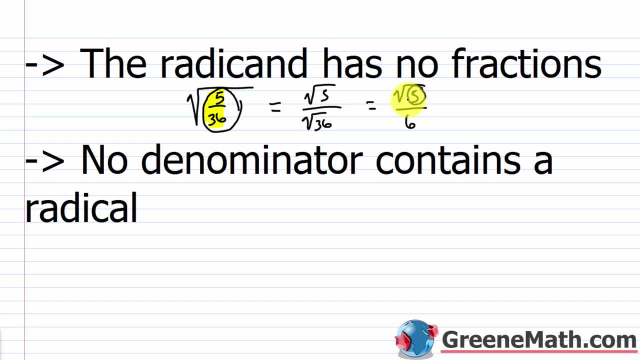 so if you see a denominator that contains a radical- most of you remember this from algebra 1- you have to use a process known as rationalizing the denominator. we're not going to get to that in this lesson, so we'll cover that kind of later on. 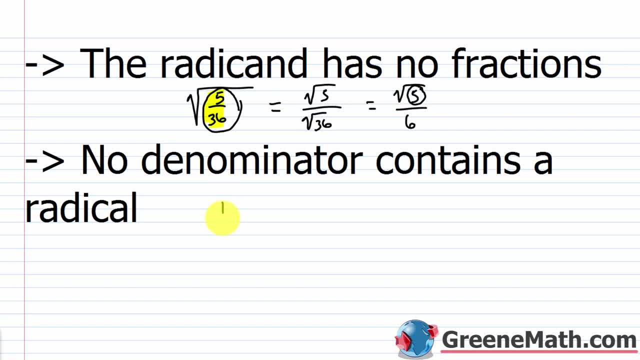 but it's a very, very simple process. if i end up with something like, let's say, 1 over the square root of 2, i just basically multiply the numerator and denominator by square root of 2, and what happens? square root of 2 times square root of 2 is 1. 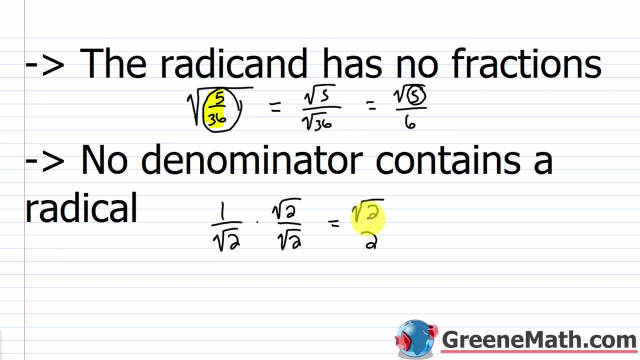 that becomes 2, then the numerator is 1 times square root of 2. so all they're saying is that versus having it in this format- 1 over square root of 2- we'd rather see square root of 2 over 2. we don't want a radical. 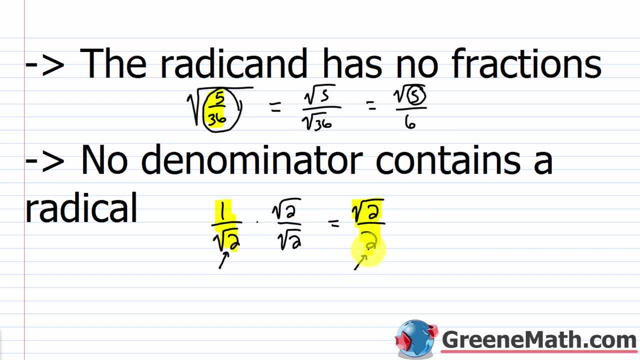 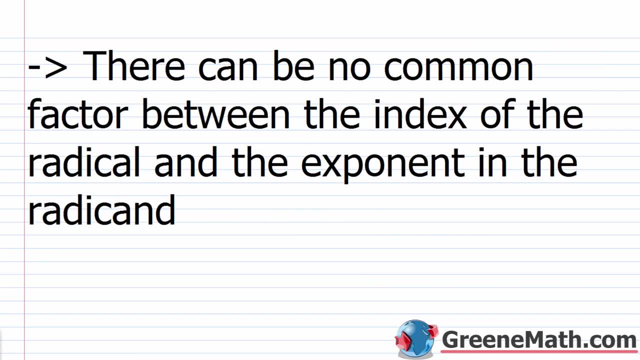 in the denominator. here there's a radical in the denominator, here it's radical free in the denominator. so this is preferred to this, although they are mathematically equal to each other. alright, then the last one we'll talk about. there can be no common factor between the index of the radical. 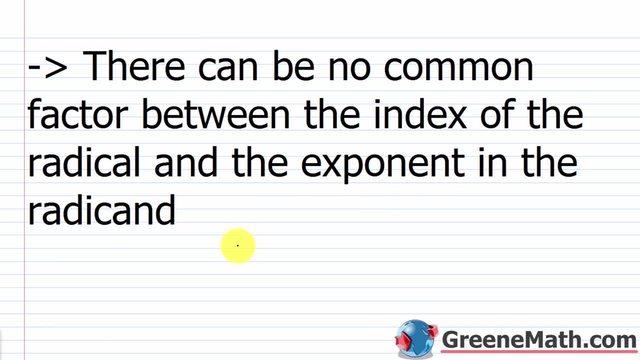 and the exponent in the radicand. so in other words, if you saw something like this, let's say you saw i don't know, the fourth root of, let's say, 4 squared. so for this one you could just convert it into exponent form and you could say: you have what? 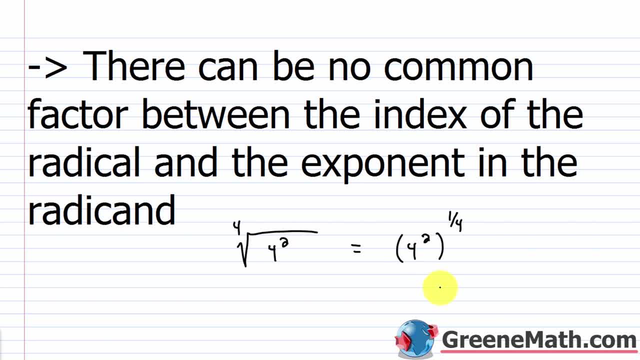 you have 4 squared, that's raised to the power of 1 fourth. now power to power rule tells you you have what you have: 4 raised to the power of 2 times the fourth, which is 2 fourths, and you can see what they're talking about. 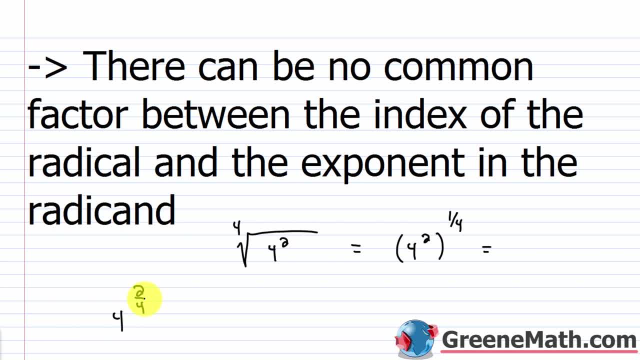 you don't want to have a fraction there that has a common factor. so let's simplify that: 2 fourths is the same as 1 half, so this is 4 to the power of 1 half, or in other words, it's the square root of 4. 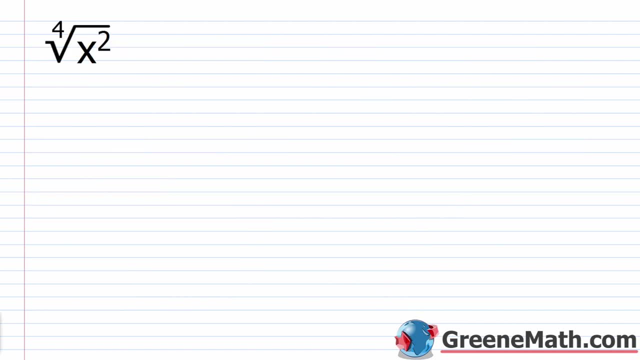 which is 2. alright, let's just run through some examples here real quick. again, this is something we talked about in algebra 1. for most of you, you'll remember this. it just comes back to you very, very quickly. for others who've never seen it, it's something you just pick up. 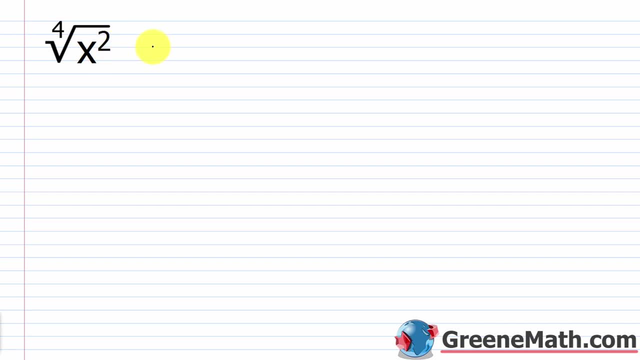 it's not a very challenging process. so we have the fourth root of x squared again. for something like this, you just write everything in exponent form, x squared, and then it's raised to the power of 1, fourth. so in this form again, if I have x, that stays the same. 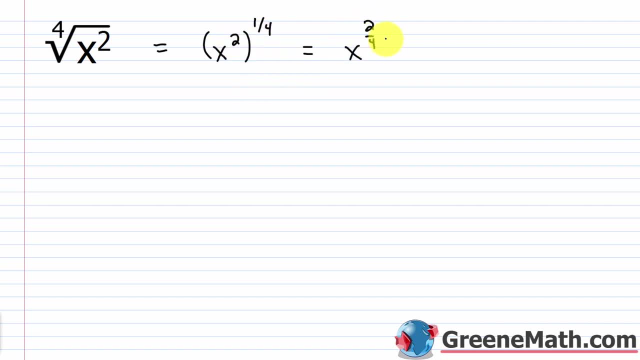 and then we multiply 2 times the fourth. we know that's 2 fourths. we just did this in the previous example, where 2 fourths was reduced to 1 half. so this is x to the power of 1 half, or, if you wanted to, you could write: 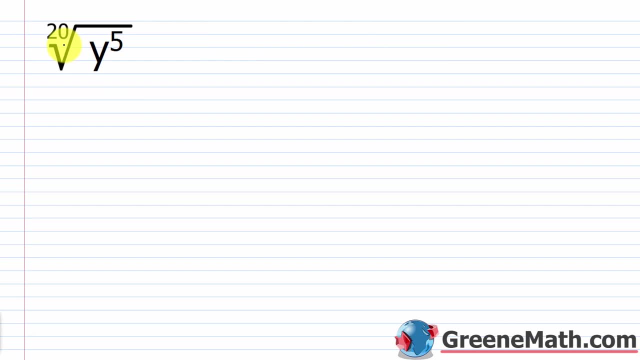 the square root of x. what about something like the 20th root of y to the 5th power? again, let's write y to the 5th power, raised to the power of 1 over 20. this index here becomes your denominator. so that's how I got that. 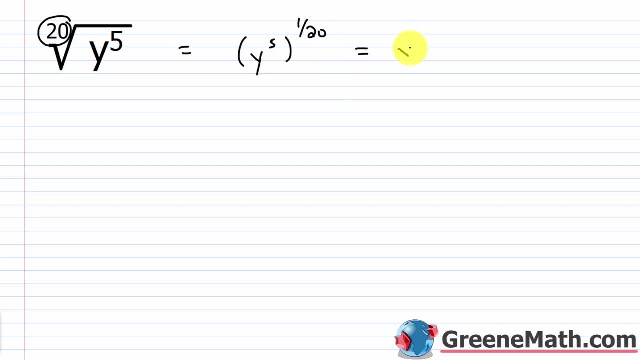 so now again, power to power. rule y stays the same. you'd multiply 5 times 1 over 20 is 5 over 20. of course, 5 and 20 are each divisible by 5, so I could reduce that 5 divided by 5 is 1. 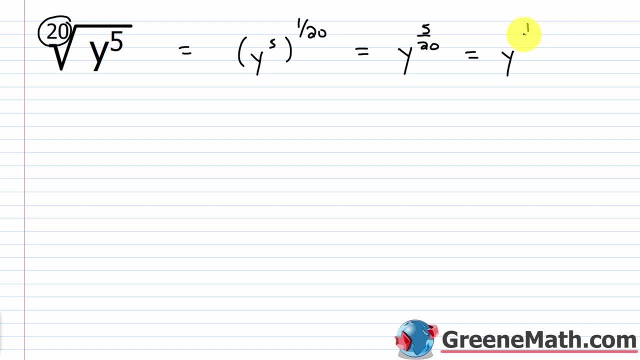 20 divided by 5 is 4. so this is y raised to the 1 fourth power. or again, this is the fourth root. again, that 4 comes from that denominator. that's where I'm getting it. so it's the fourth root of y. so now let's take a look at. 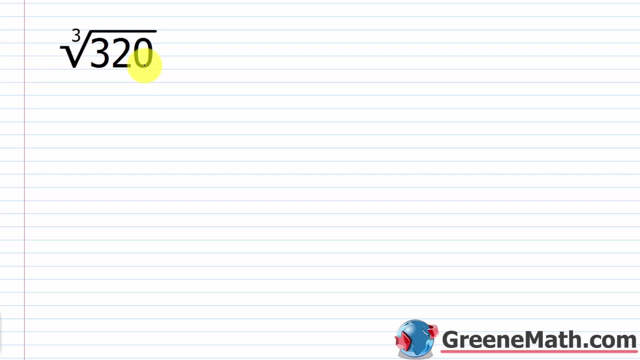 the cube root of 320, and we just want to simplify this. so what we're going to do is we're going to factor 320 and we're going to look for perfect cubes, because this is a cube root. if I had a fourth root, I'd look for a perfect fourth. 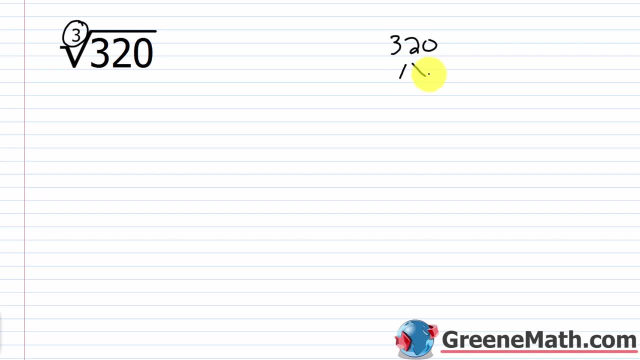 if I had a square root, I'd look for a perfect square. so, factoring this, what can you tell right away? we're going to multiply 10, so this would be 32 times 10. now, without going any further, a lot of you remember that 32 is what. 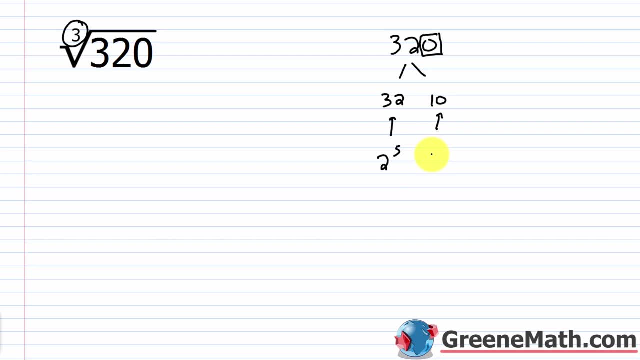 it's 2 to the fifth power. 10 is 2 times 5, so really 2 to the fifth power times 2 is 2 to the sixth power, so this is 2 to the sixth power times 5. now let's just stop for a minute. 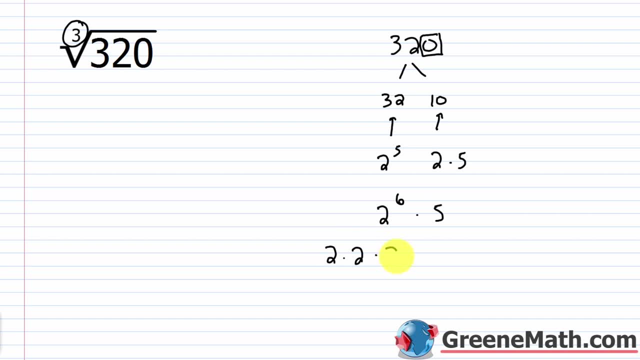 let's write out 2 to the sixth power, so it's 2 times 2 times 2 times 2, so I can put this into 3 groups of 2 times 2, because this would be a group and this is 4. this would be a group and this is 4. 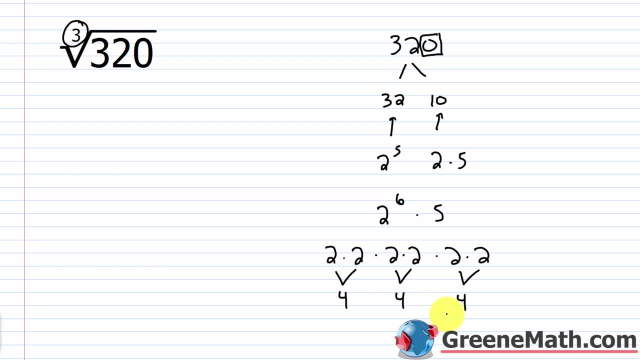 and this would be a group, and this is 4. that's exactly what I'm looking for. I'm looking for a perfect cube, and the perfect cube would be 4 times 4 times 4, which is 64, so I can write this as what? 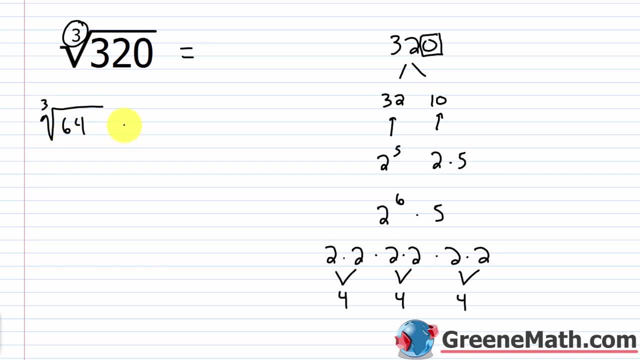 the cube root of 64 multiplied by the cube root of 5. now, the cube root of 5 is not going to be able to be simplified any further, but what we're saying is that we could replace this with a 4. cube root of 64 is 4. 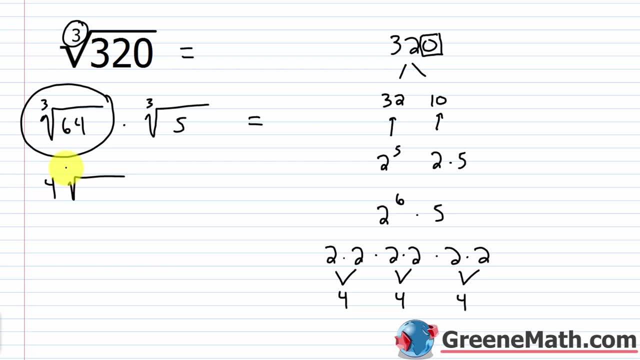 so why not just write a 4 there? then we put times the cube root of 5. so that's your simplified answer. now, another way to do this. let's kind of erase this real quick, and in my opinion it would be a little bit quicker. you could do this using exponents. 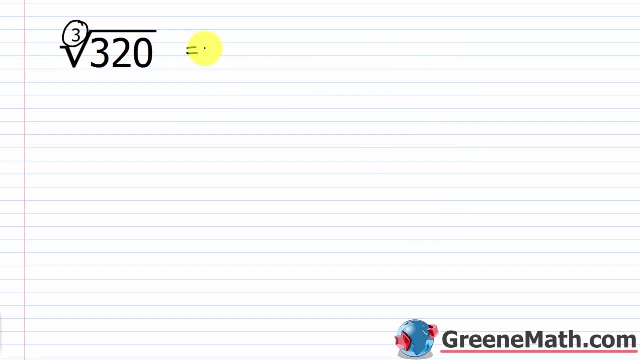 so let's say that you want to just start out by saying: okay, this is 320 raised to the power of 1 third. now if you realize that this is 64 times 5, and 64 is 2 to the 6th power, you could say: okay, 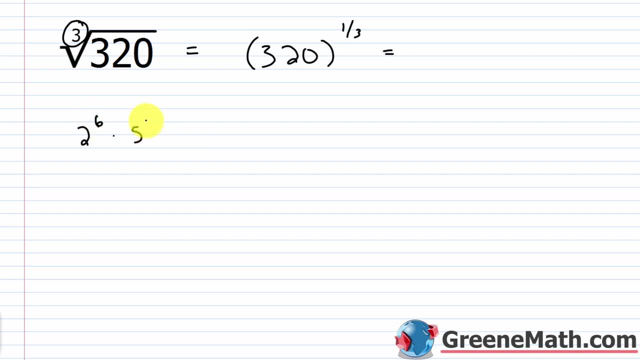 well, I could write this as: 2 to the 6th power multiplied by 5, this is all raised to the power of 1 third. again, all I'm doing is just using rules that we learned back when we talked about exponents, so I can further break this down. 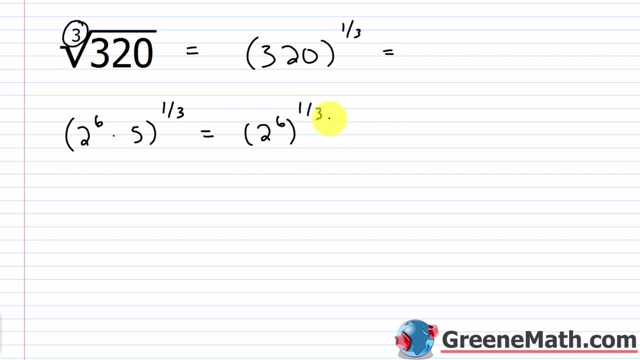 into 2 to the 6th power. raised to the power of 1 third, multiplied by 5 raised to the power of 1 third, I can use my power to power rule and say 2 to the 6th power is raised to the power of 1 third. 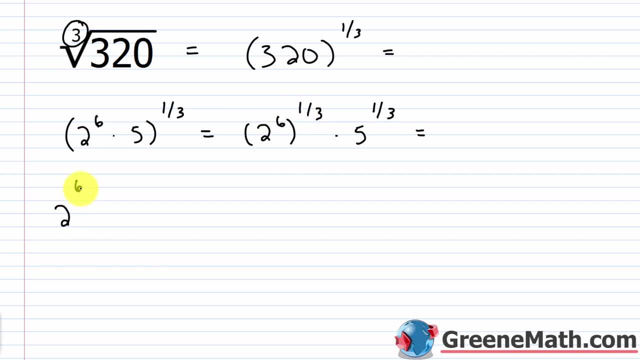 that would be 2 raised to the power of 6 thirds, then multiplied by 5 raised to the power of 1 third. now 6 over 3 is 2. so this would give me 2 squared times 5 to the power of 1 third. 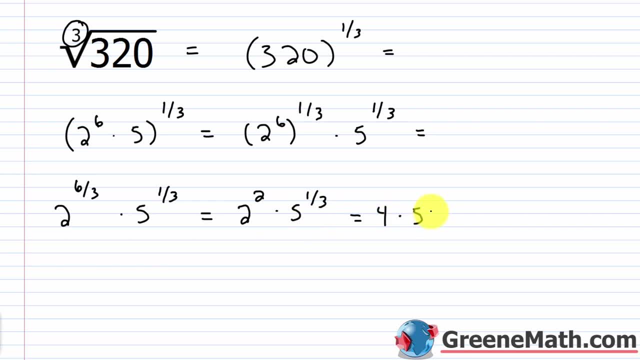 we know, 2 squared is 4 be 4 times 5 raised to the power of 1 third, And 5 raised to the power of 1 third is the cube root of 5.. So this is nothing more than 4 multiplied by the cube root of 5, which is exactly what we. 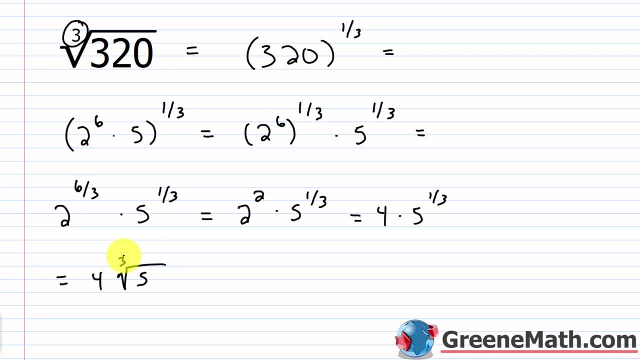 just saw a minute ago. So kind of: either way, you want to do this. A lot of times I personally like to use exponents because they're a little bit quicker for me, But if you want to do it the other way, that's fine too. Again, you're just trying to get the right answer. All right, as 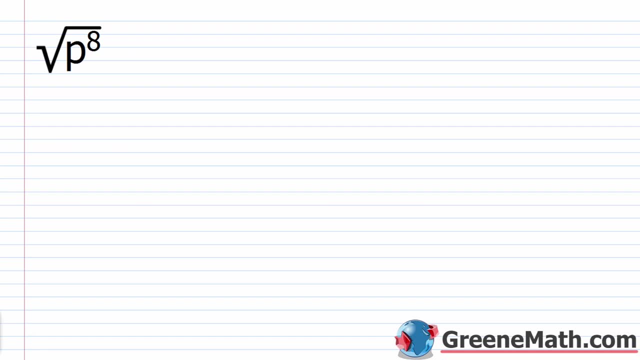 another example. let's say we looked at the square root of p to the 8th power. This is a good one to do with exponents. So we would say we have p to the 8th power and this is raised to the. 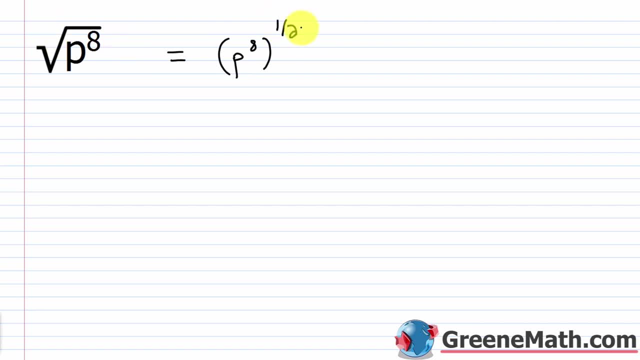 power of 1 half. Remember, if you have the square root of something, it's like having the radicand raised to the power of 1 half. So, using my power to power rule, I'd have p raised to the power of. 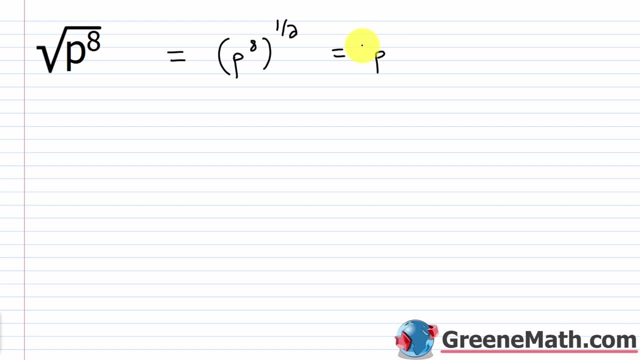 8, and then that's raised to the power of 1 half. So p stays the same. We multiply 8 times 1 half, That's 8 over. So this is p to the 4th power. All right, p to the 4th power, All right. let's take a look at. 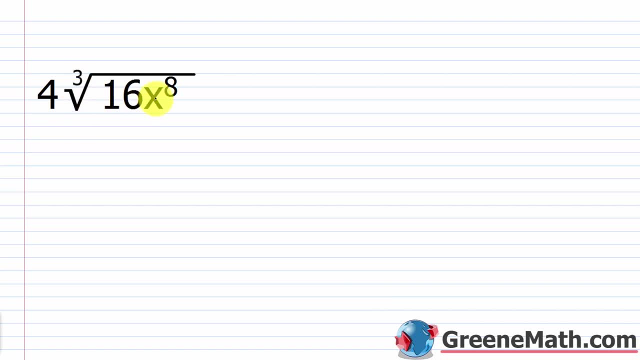 another one. So we have 4 multiplied by the cube root of 16x to the 8th power. So let's go ahead and take 16 and factor it. We know this is what 4 times 4.. We know 4 is 2 times 2.. So we know. 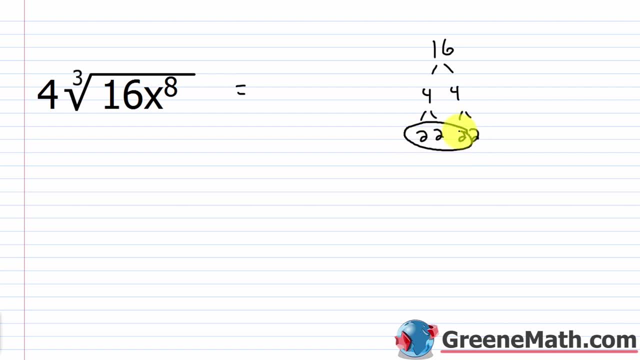 for a perfect cube we would take 3 of these and we would say it's 8 times 2.. So let's put that we have 4 multiplied by the cube root of 8, multiplied by the cube root of 2.. So I've separated. 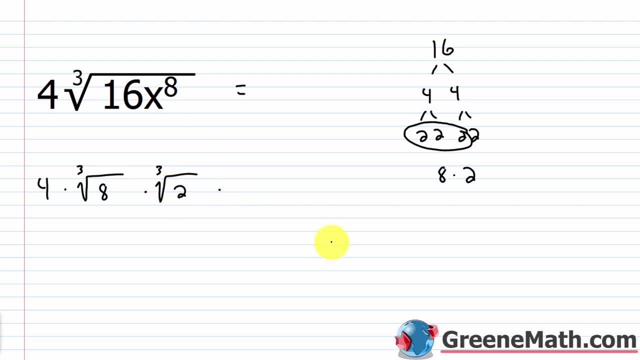 those two then multiplied by. Then the next thing I come across is this: x to the 8th power. So to figure out the perfect cube there, look at the exponent. there The exponent is an 8.. The index here is a 3.. So you've got to think about what's the closest thing to 8 going down, that's going to. 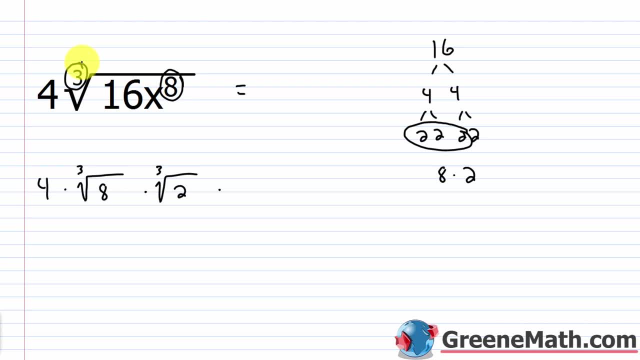 be divisible by 3.. Well, that's going to be 6.. So, in other words, I would split this up into: the cube root of x to the 6th power times. the cube root of x squared x to the 6th power times x squared is x to the 8th. 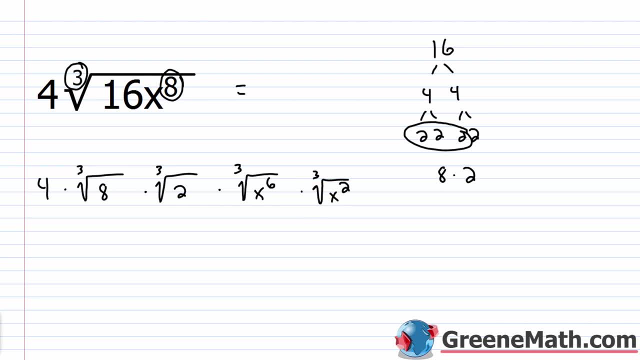 power. So once this is all broken down, we can further simplify this and this. But then when we look at these two, this one and this one- we're not going to be able to do anything else. So in other words, you will have 4 multiplied by the cube root of x to the 6th power. So that's going to. 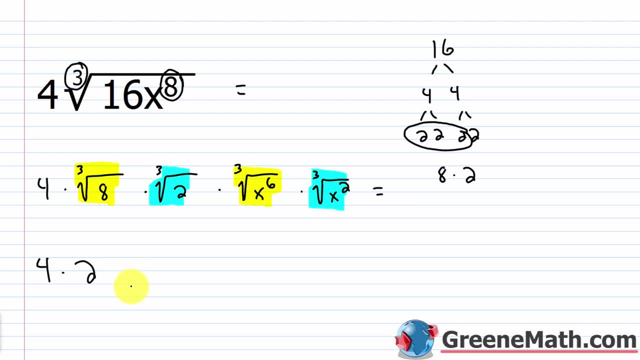 be: 4 multiplied by the cube root of 8 is 2.. And then the cube root of x to the 6th power. All you really have to do is divide. here You say 6 divided by 3 would be 2.. Another way to do that: 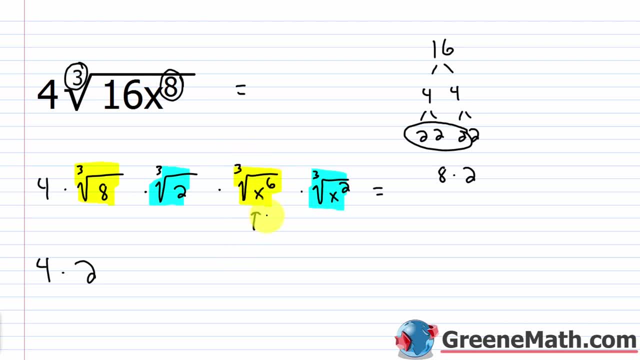 again. if you're uncomfortable doing that, just go ahead and write that off to the side. using exponents, You have x to the 6th power raised to the power of 1 third. You know this would end up being what. x stays the same. Multiply exponents 6 times 1 third is 6 over 3.. 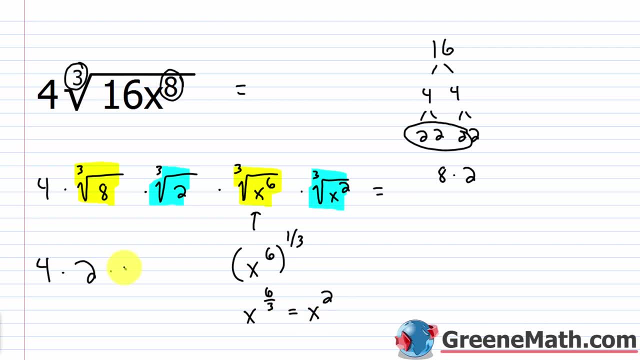 And 6 over 3 is 2.. So this is x squared. And again, that's the reason why I asked the question: what's the closest number to 8?? Again, it's got to be going down, It can't be going up. 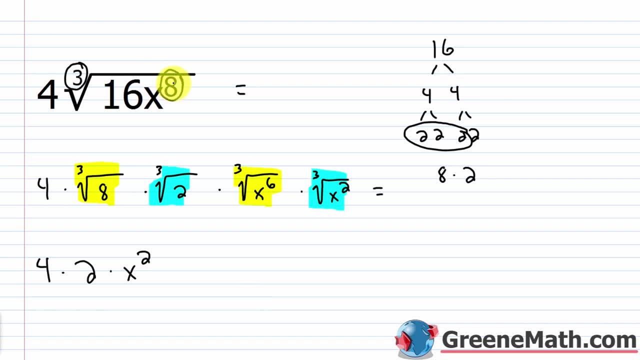 We can't go into 9 or 10 or something like that. We don't have that, So we have 8 of these. What's the closest number going down? That's divisible by 3. It's not 8.. It's not 7.. 6 is. 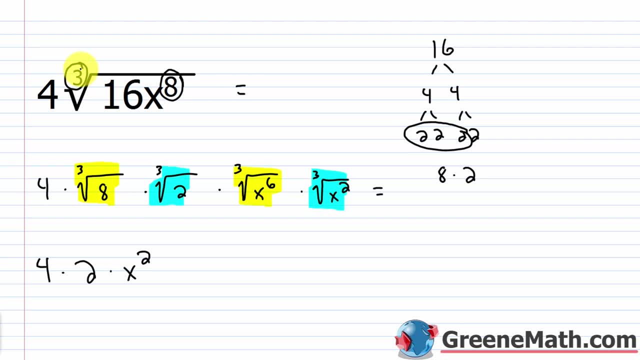 divisible by 3.. So that's kind of what you're doing in your head. Then the next thing we have: we have this cube root of 2. Which can't be simplified, And this cube root of x squared, which can't be simplified Because 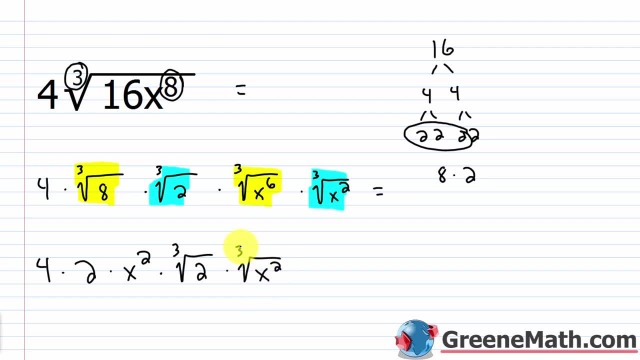 you think about x squared there. there's not enough x's to have a perfect cube, right? If I had x cubed, that'd be a perfect cube. It'd be x times x times x. But I just have x times x It's. 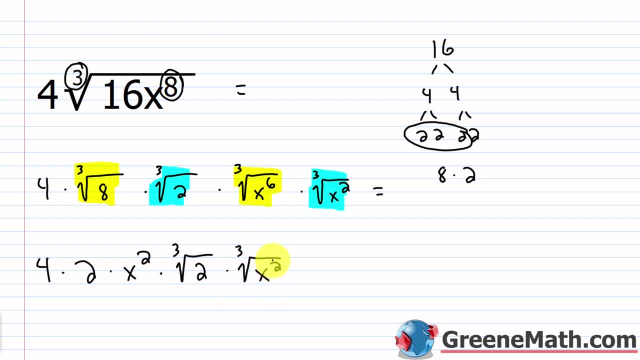 not enough to have a perfect cube, So that can't be simplified. So now all I do is multiply things together. on the front, 4 times 2 is 8. Then times x squared. So that was what we could take out. 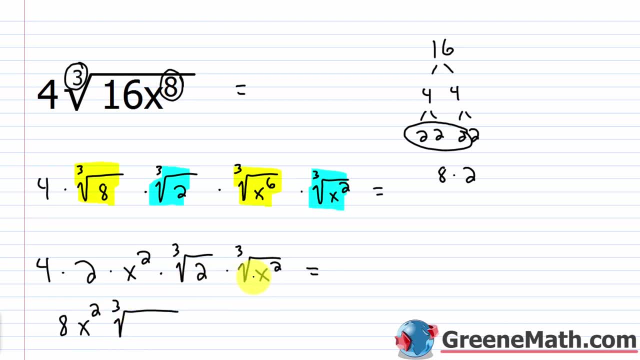 Then what's left? we'd have the cube root of 2 times x squared, or just 2x squared, And just notice how inside here your radicand. you can't simplify that any further. 2 is not a perfect cube and 2 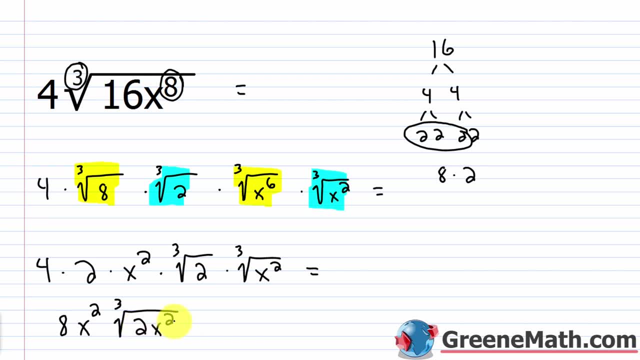 doesn't factor right, It's just 2 times 1.. x, squared again, as we just talked about, is not a perfect cube, So you can't do anything further with this. So you just report your answer as 8x. 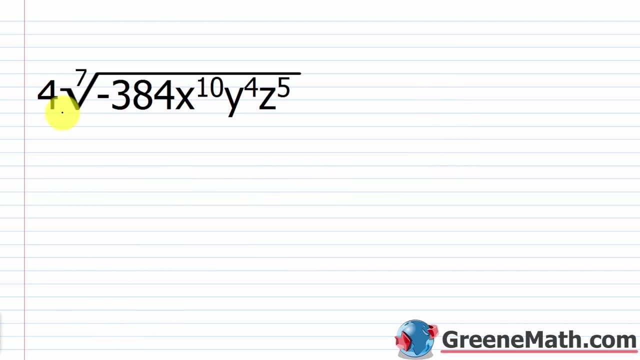 squared times the cube root of 2x squared. All right, for the next one we're going to look at one that's kind of tedious. We have 4 times x squared, So that's 2 times x squared. So that's. 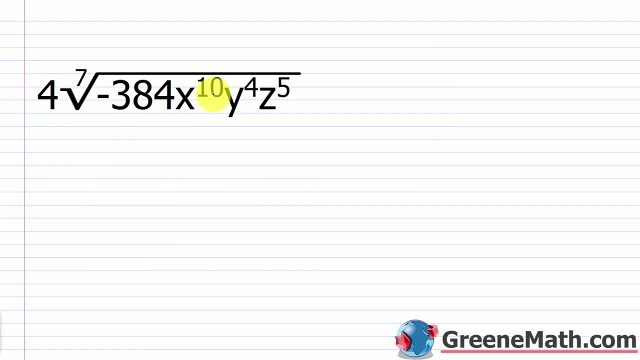 4 times the seventh root of negative 384,: x to the 10th power, y to the 4th power, z to the 5th power. So what can we simplify right away? So we have 4 multiplied by, we have the seventh root of. 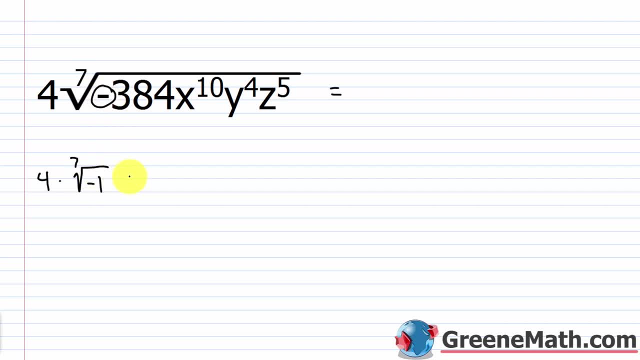 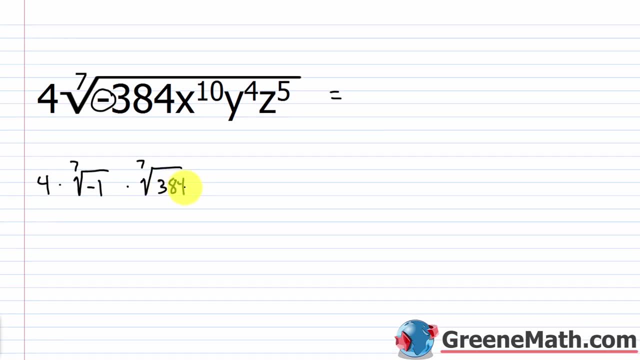 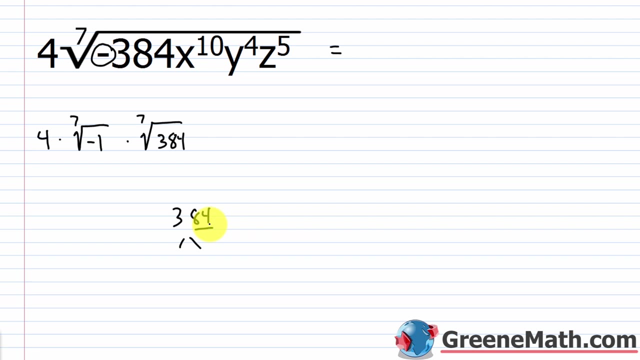 what? Let's deal with this negative. I can put the seventh root of negative 1 multiplied by the seventh root of 384.. And we can deal with that number part. right now We do a factor tree. Notice that the final two digits- 84, are divisible by 4.. So therefore the number is 384 is 4 times. 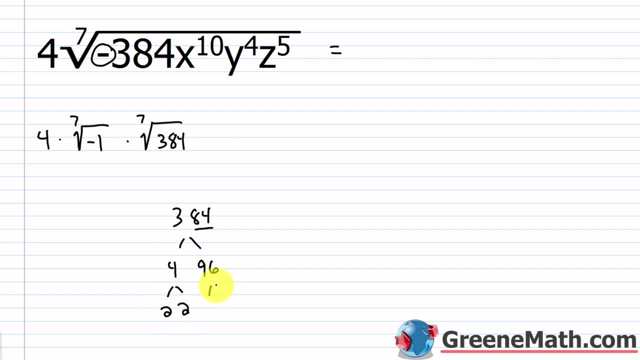 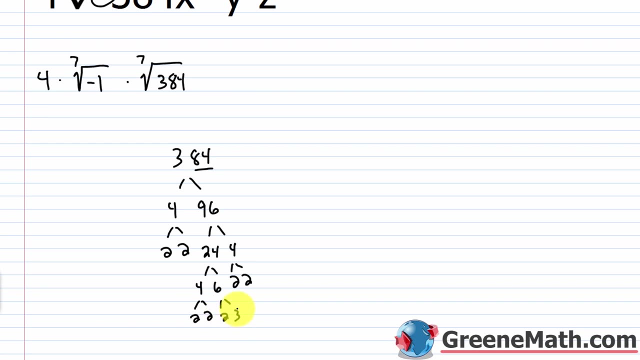 96.. Now 4 is 2 times 2.. 96 is what It's also divisible by 4. It's going to be 24 times 4.. 4 again is 2 times 2.. 24 is 4 times 6.. 4 is 2 times 2.. 6 is 2 times 3.. So you've got 1,, 2,, 3,. 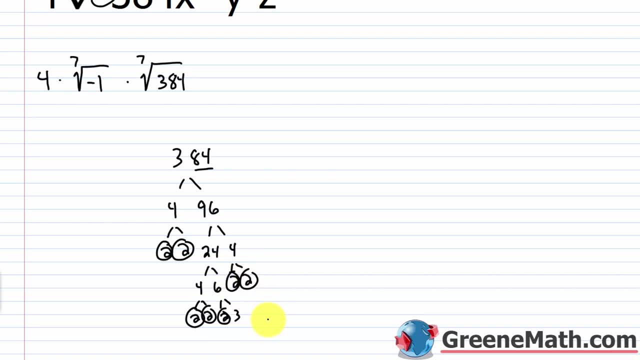 4, 5, 6.. 7 factors of 2 times 1 factor of 3.. So this is 2 to the 7th power times 3.. So let's write this as the seventh root of 128, which we know is 2, times the seventh root of 3.. Now we're not going. 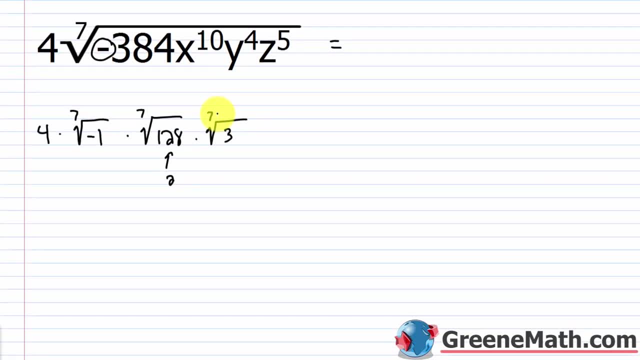 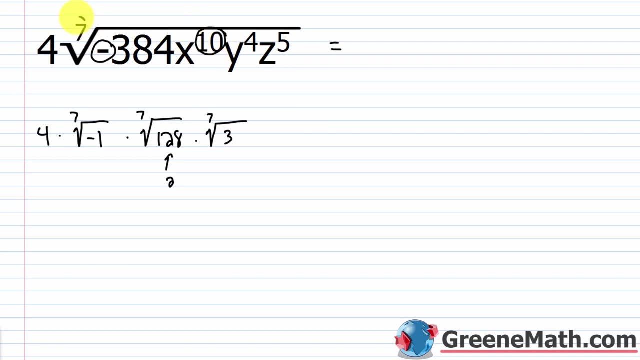 to be able to simplify this any further. So we would just end up leaving that as it is. Then we deal with the variables here. Now if I have an exponent that is greater than or equal to this index, here I want to pull enough out to where I can simplify. So if I have x to the 10th and I have 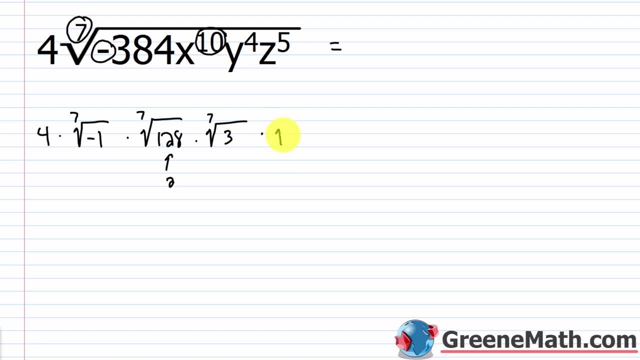 a seventh root. what I want to do is I want to split this up into the seventh root of x to the 7th, because that would simplify. then multiplied by the seventh root of x, cubed x to the 7th times. 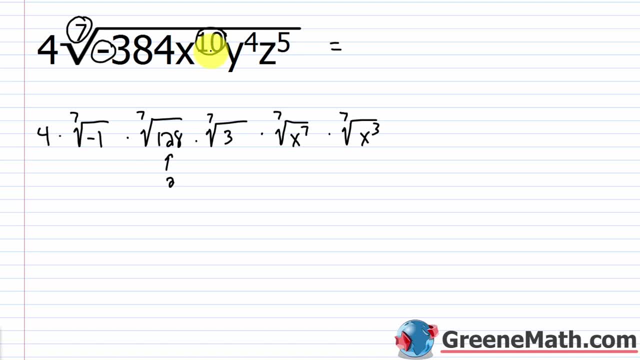 x cubed is x to the 10th. That's all I did there. Then, multiplied by, you'd have the seventh root of y to the 4th. You can't simplify this. You can't simplify this. You can't simplify this, You can't. 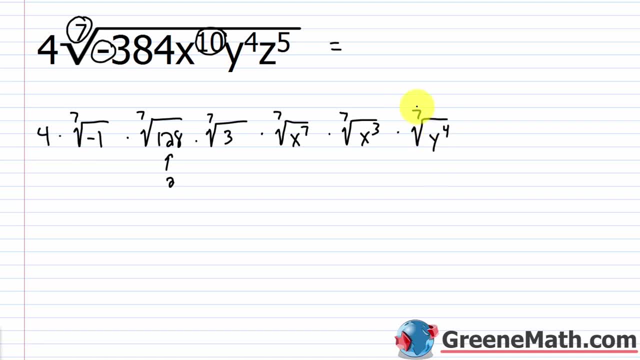 simplify that, because 4 is smaller than 7.. There's just not enough. Then, multiplied by the seventh root of z to the 5th, Same thing. The 5 is smaller than the 7, so there's not enough The reason we could. 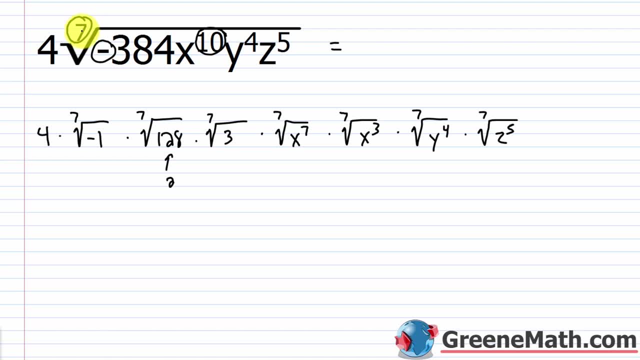 simplify: the 10 is because it was greater than the 7.. So I pulled 7 out. That's what this is here. And then 10 minus 7 is 3, so that's how I got this 3 here. So now, what can we simplify? We can. 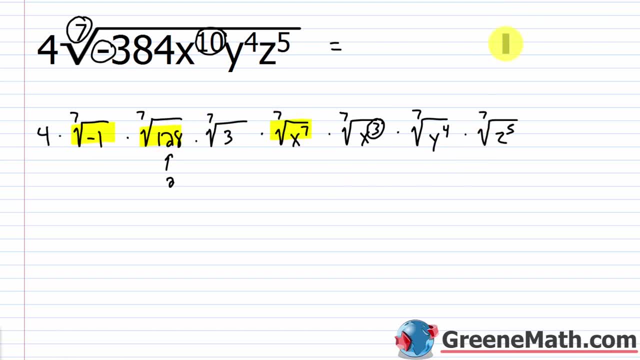 simplify this and this and this, Everything else we can't. So if I think about the seventh root of negative 1, that's just negative 1.. So you'd have negative 1, multiplied by you have a 4 there. The seventh root of 128 is 2.. And then let's do this one, The 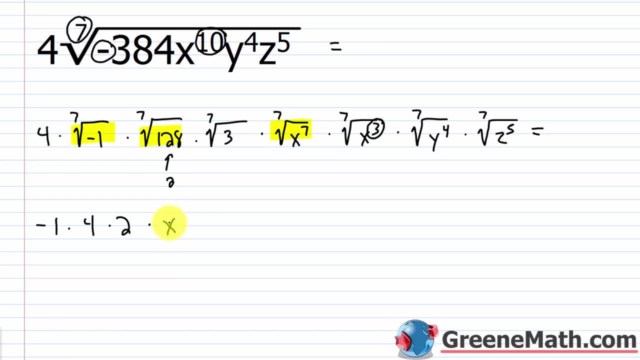 seventh root of x to the 7th power is just x, right? Because x times itself 7 times is x to the 7th power. So those are pulled out to the front And then we have everything else that we'll just combine. So times we'll have the seventh root of 3, then times. 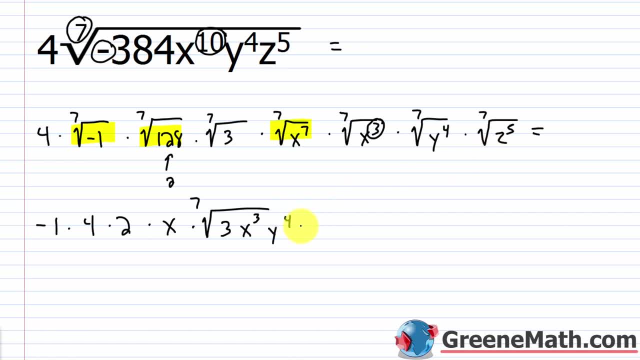 x cubed, then times y to the 4th, then times z to the 5th. And the easy way to tell if you've simplified something when you have variables involved: just look at the exponents Again. if the exponents are smaller than the index, you're good to go right. This is a 3,. this is a 4,. 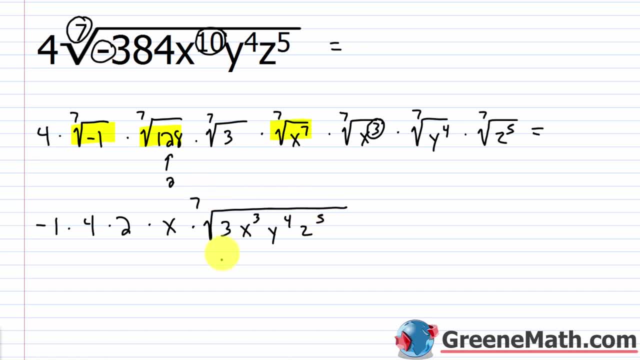 this is a 5. They're all smaller than 7.. As far as the number part goes, you can look at 3 and say 3 is a prime number. There's nothing I can do there, So what I'm left with? 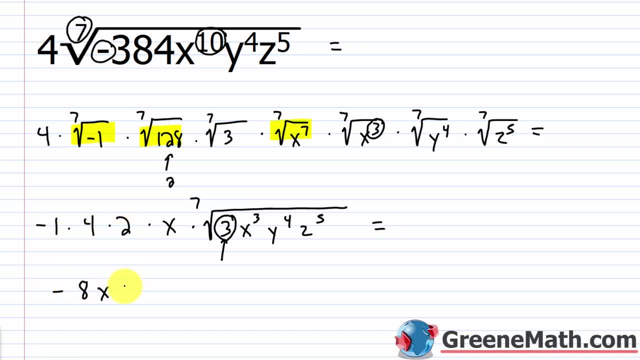 1 times 4, times 2 is negative 8, then times x, then times the 7th, root of again 3x, cubed times y to the 4th, times z to the 5th. All right, so the last thing I'm going to cover. 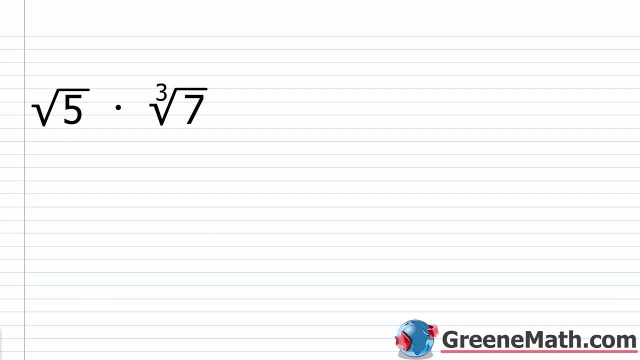 today we're going to talk about how we simplify products and quotients of radicals with different indexes. So a lot of students don't even know this is possible, but this is definitely something you can do. So if I have something like the square root of x, I'm going to have a square root of x. 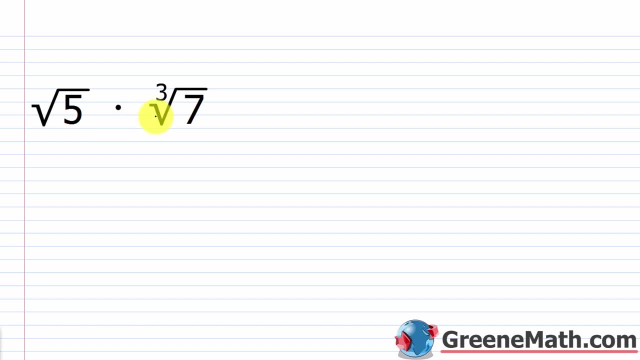 I'm going to have a square root of 5 multiplied by the cube root of 7.. What could I do here? I can't just say, oh, you know, square root of 5 times 7.. Sometimes you'll see students go, okay. 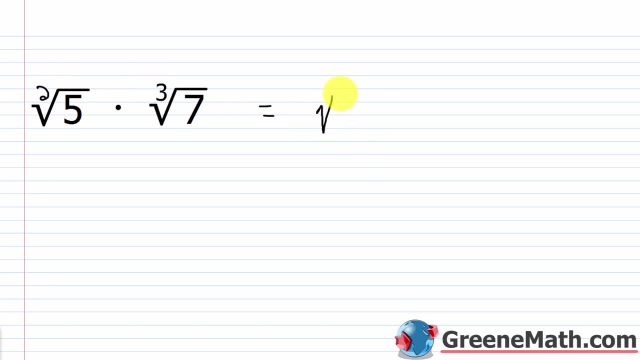 well, that's, this is a 2,, this is a 3.. 2 times 3 is 6, so it's the 6th root of 5 times 7.. Those are wrong, okay. What you need to do is convert this into exponent form, So you basically have. 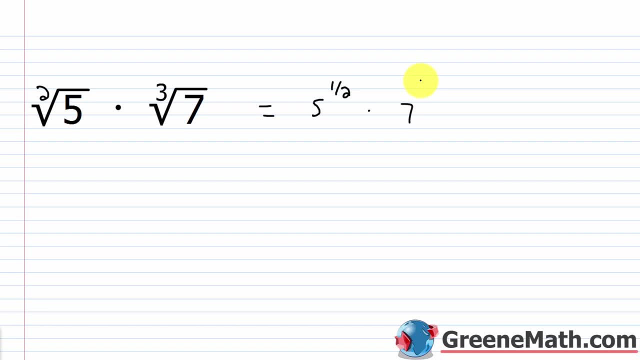 5 raised to the power of 1 half, multiplied by 7 raised to the power of 1 third, Then you're just going to get a common denominator goal. That's all you need to do. So if I have something like 1 half and I have 1 third, the common denominator would be a 6,. 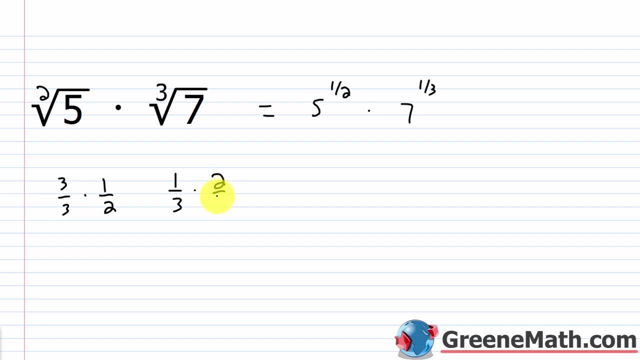 right, I'd multiply this by 3 over 3,, multiply this by 2 over 2, and I'd end up with what? 3, 6, and I'd end up with 2, 6.. So all I would do is write this as 5, and that would be raised to. 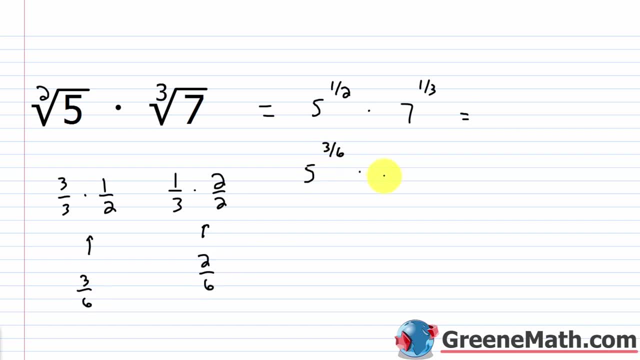 the power of 3, 6, and then times you'll have 7. Raised to the power of 2, 6.. So the index would be the same. If I convert this back into kind of a radical, I will now have the 6th root of 5 cubed multiplied by the 6th root of 7 squared. 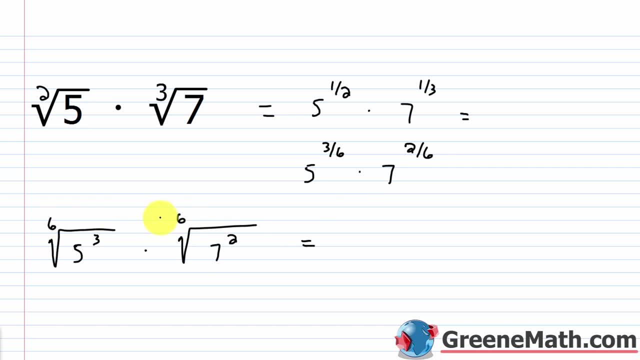 Now I have the same index here. Now I can use my little trick. I can say: this is the 6th root of 5 cubed, which is 125.. Multiplied by the 6th root of 7 squared, 7 squared is 49.. 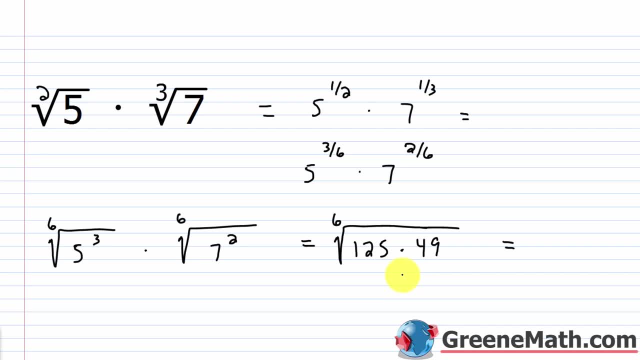 Now, this is a really big number in here, but at least we can combine it this way. So if you do 125 times 49, it's 6,125.. So we'd have the 6th root of 6,125.. 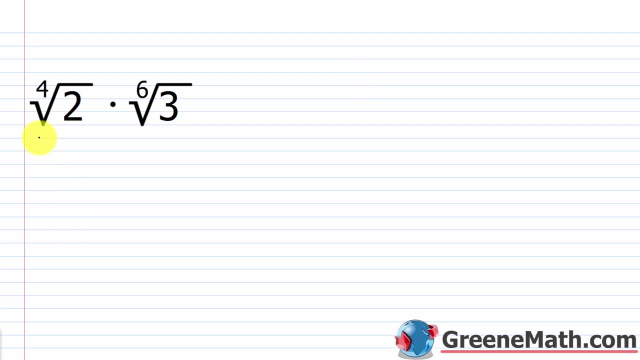 Well, let's take a look at one more example like this. So suppose you had the 4th root of 2 multiplied by the 6th root of 3.. Again, I would just multiply this by the 6th root of 3, and I'd end up with 6,125. 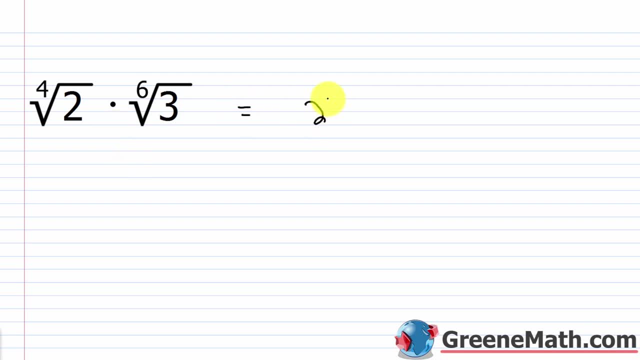 So if I had the 6th root of 2 multiplied by the 6th root of 3, I'd end up with 6,125.. I'd just write this in exponent form. I would say: this is 2 raised to the power of 1, 4th. 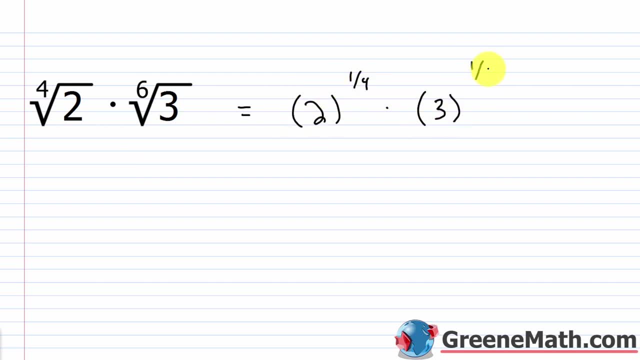 multiplied by 3, raised to the power of 1- 6th. And then we just think about what, Between 1, 4th and 1, 6th, the common denominator, the least common denominator, to be more specific, would be: 4 is 2 times 2.. 6 is 2 times 3.. So you'd basically have: 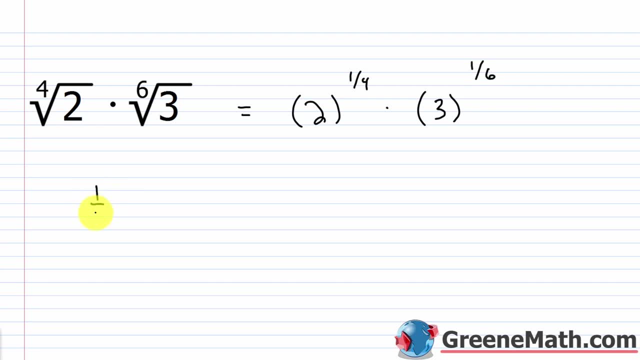 2 times 2 times 3, or 12.. So I would multiply 1 4th times 3 over 3.. I would multiply 1: 6 times 2 over 2.. So 1 times 3 is 3 over 4 times 3, which is 12.. Over here, 1 times. 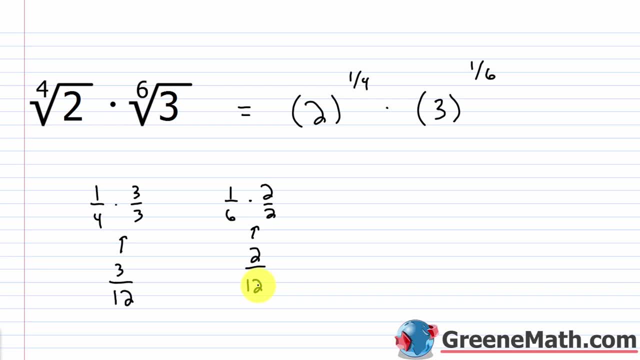 2 is 2 over 6 times 2, which is 12.. So 3 twelfths and 2 twelfths. So I would write this, as we'll have 2 raised to the power of 3 twelfths multiplied by 3 raised to the. 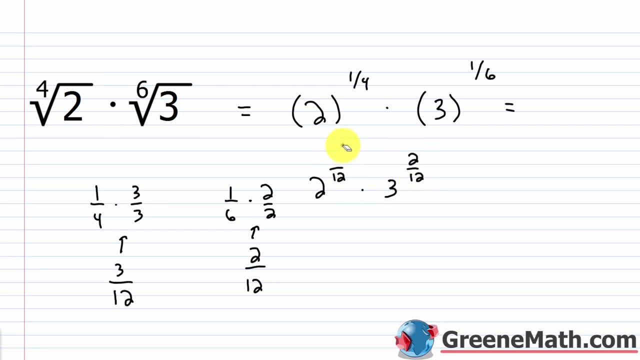 power of 2 twelfths. Let's erase this. Let's erase this. So now, looking at it, I can rewrite it, I can go back into radical form. This is going to be the 12th root of 2 cubed multiplied. 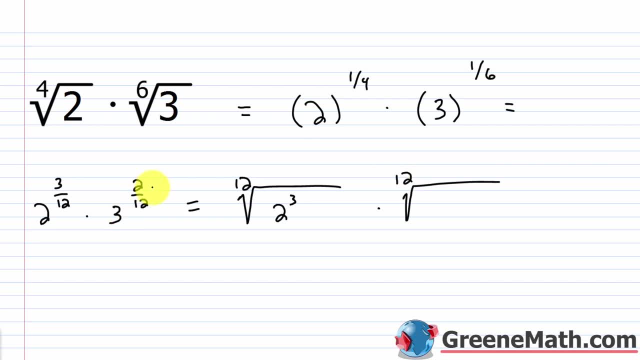 by the 12th root of 3 squared. So this equals what We'll have. the 12th root of 2 cubed is 8.. So this equals what We'll have. the 12th root of 2 cubed is 8.. 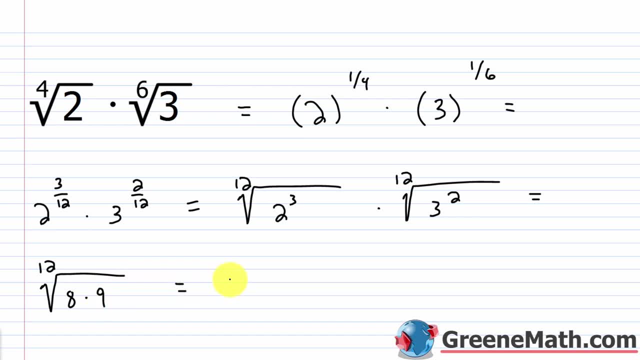 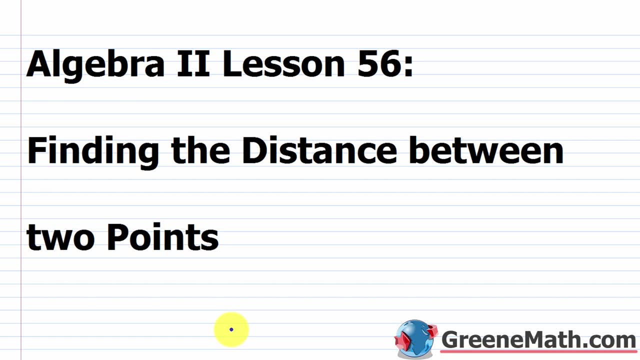 So this equals what We'll have. the 12th root of 2 cubed is 8.. Multiplied by 3 squared, which is 9.. This will end up being the 12th root of 72.. Hello and welcome to Algebra 2, Lesson 56.. In this lesson, we're going to learn about 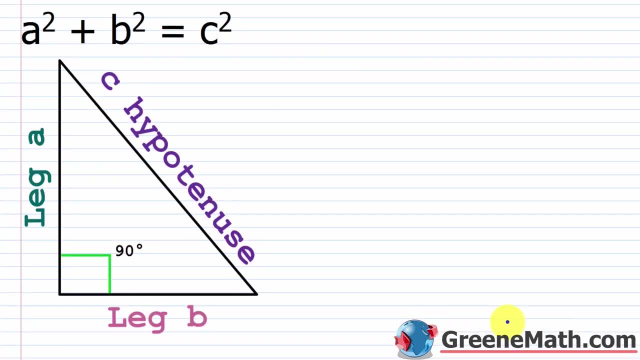 finding the distance between two points. So again we have another topic that we covered back in our Algebra 1 course. So for most of you, this lesson will just be a review. If you haven't seen this topic before, don't worry, This lesson is going to be very, very 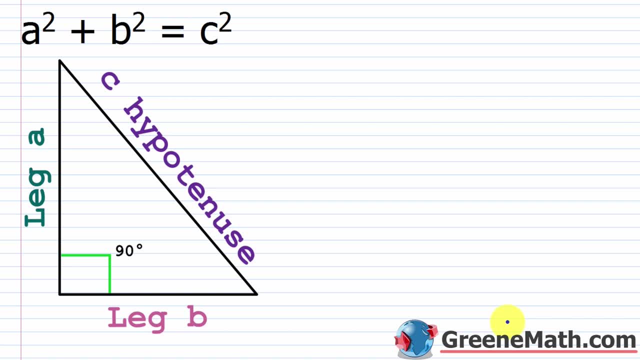 easy. This concept is something you can pick up pretty much right away. So, again, the idea is just to be able to figure out the distance between any two points on a coordinate plane, And basically the way we're going to do this is we're going to use something. 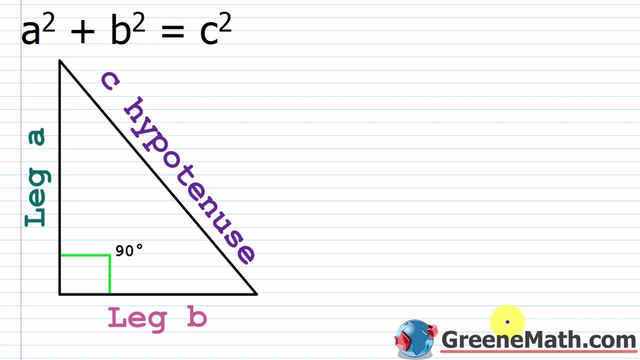 known as the distance formula. Now I know some of you will hear the term distance formula and you're immediately thinking about the distance formula we used with motion word problems. right, You're thinking about. distance traveled equals the rate of speed times. the. 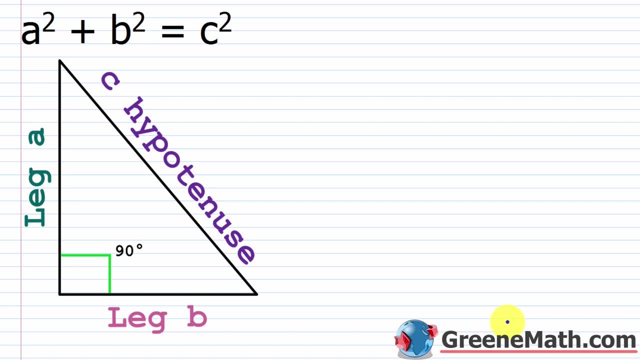 time traveled. So this distance formula has the same name, but it performs a very different application, okay? So, essentially, you're going to pick one of the points and you're going to choose a number. So you're going to pick one of the points and you're going to. 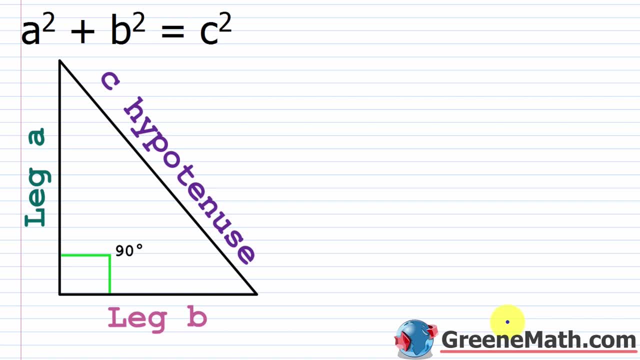 choose it to be x sub 1, y sub 1.. You're going to pick another point. You're going to choose it to be x sub 2, y sub 2.. And you're going to plug into this formula and it's going: 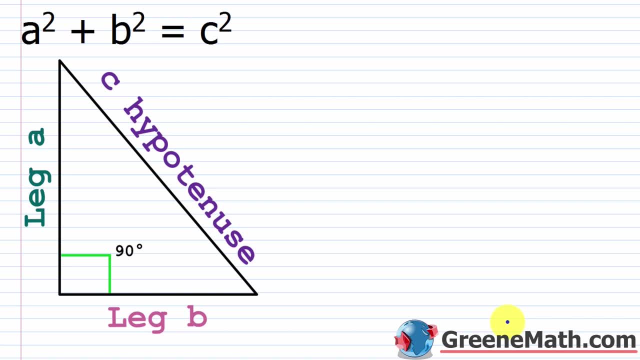 to spit out a distance between the two points. Very easy to use. But before we kind of get to that, I want you to understand where it comes from. So basically, it's a direct application of the Pythagorean formula, or you could say the Pythagorean theorem. So that's the very 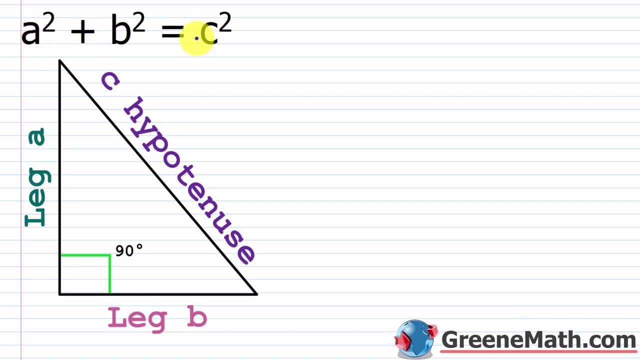 famous a squared plus b squared equals c squared that you see on your screen. So the Pythagorean formula basically relates the lengths of the distance between two points on a coordinate of the sides of a right triangle. So you might not have taken a geometry class before. 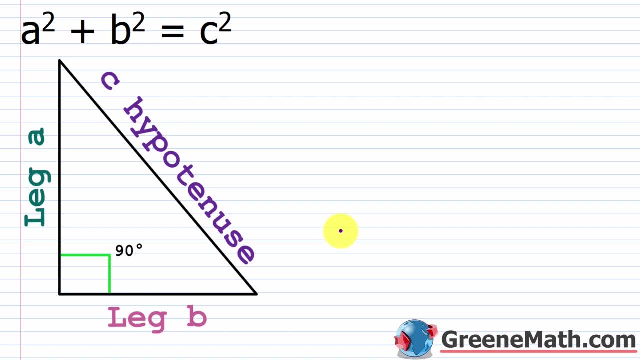 In case you haven't. basically, a right triangle is a triangle with a 90-degree angle. So this symbol right here tells you that you have a 90-degree angle or a right angle, which is why we call this guy a right triangle. So this is a right triangle, okay? So when? 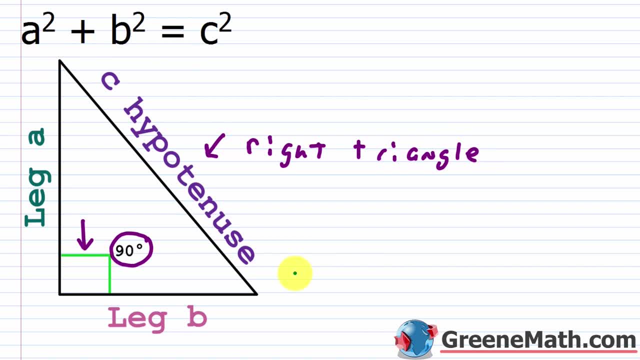 you see this symbol, you know that this formula is going to apply. So with a right triangle, we have two legs, which are normally labeled as a and b. Now, these are going to be the two shorter sides of the triangle. So you see, we have leg a here and leg b here. Then 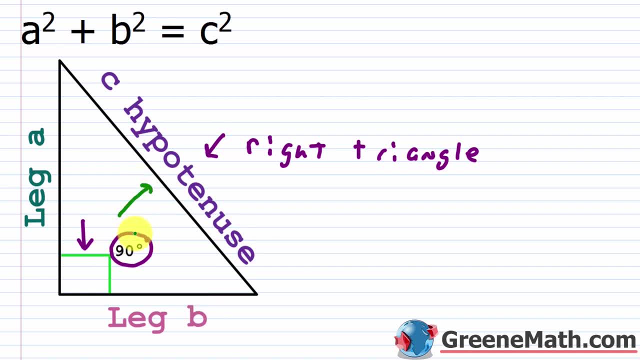 we have the longest side, which is always opposite of this 90-degree angle. This is known as the hypotenuse and this is always going to be labeled as c. So essentially, when we square each of the two legs and then sum those amounts, it's always going to be. 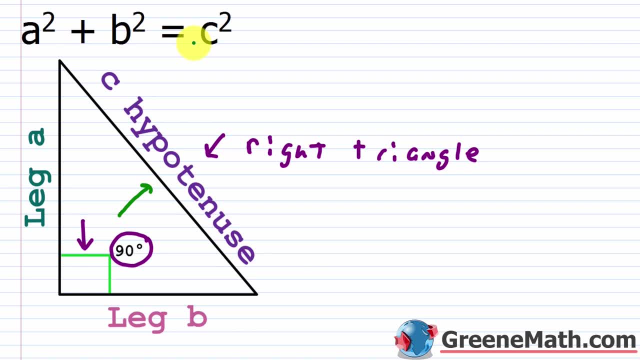 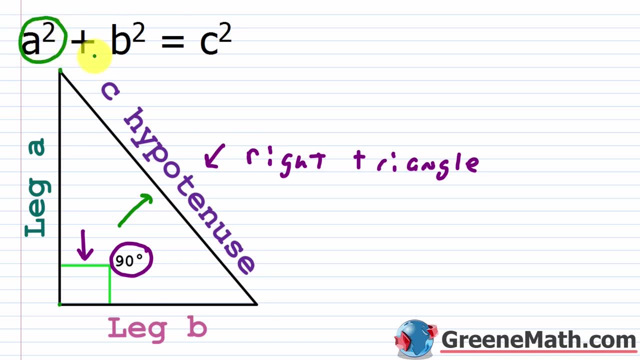 equal to the hypotenuse squared, So in other words the measure of leg a. so from here to here, if I square that guy, that's where I get this a squared from. and then I add that to the measure of leg b. so from here to here, that guy squared, so that's where. 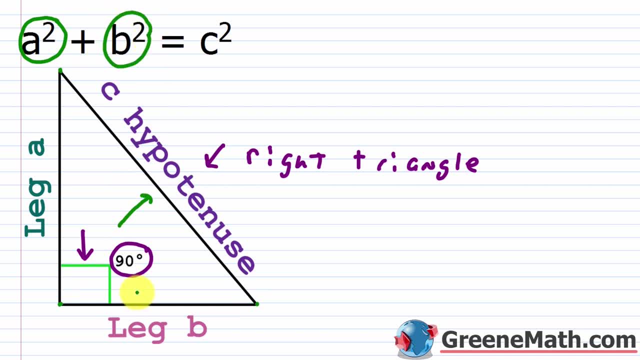 b squared comes from. this is equal to, or the same as the hypotenuse or c squared. so from here to here, okay, So that's where the c squared comes from. So a squared plus b squared equals c squared. So how can we use this to basically find out the distance? 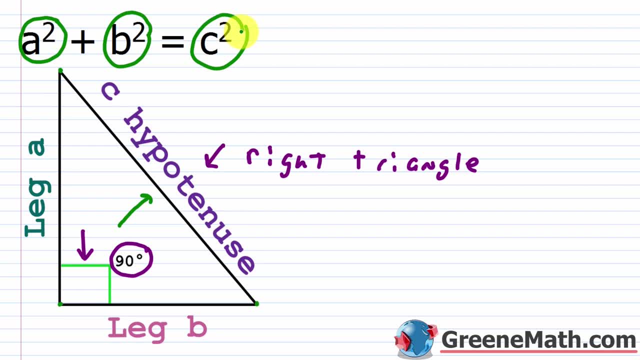 between two points on a coordinate plane. Well, what's going to end up happening is, if I square two of the sides, you can use this formula to find the third side, or basically what's unknown. So let's say, I had a point that was here and a point that was here, So 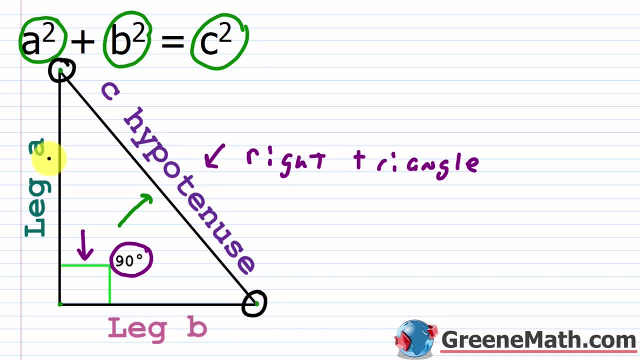 what's going to happen is I'm going to be able to find the measure of leg b and the measure of leg a. The measure of leg b will just be a horizontal distance, so from here to here, okay, So we're going to be looking at the x values for that and we'll talk about. 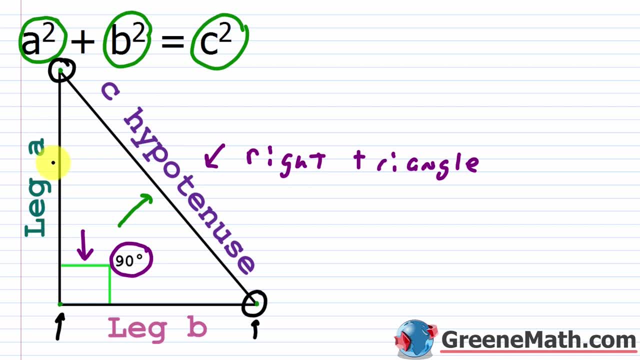 that in a minute when we get to the kind of example and then the measure for leg a, that's going to be this vertical distance From here to here. okay, so that's going to be us looking at kind of the y values, Those. 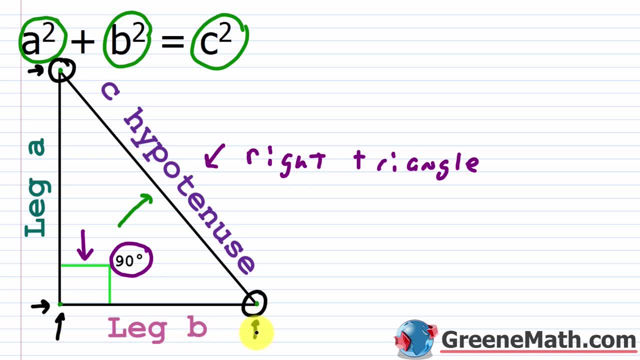 are easy to find. We can easily find the value for leg b, We can easily find the value for leg a. so we can plug that into the formula and solve for the unknown, which is going to be c, the hypotenuse, or again, in this case, the distance between the two points. 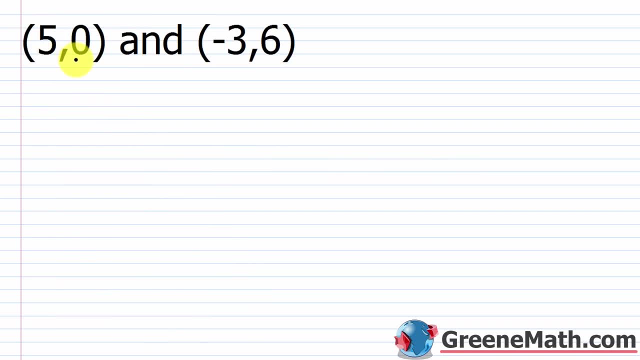 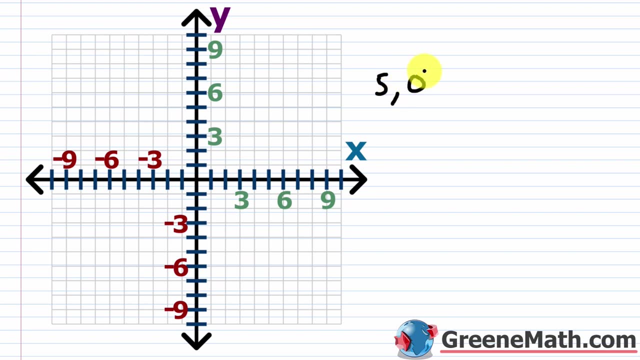 All right. so let's take a look at the example. So we have the point 5 comma 0 and the point negative, 3 comma 6.. So let's start by just plotting those. So we have 5 comma 0 and 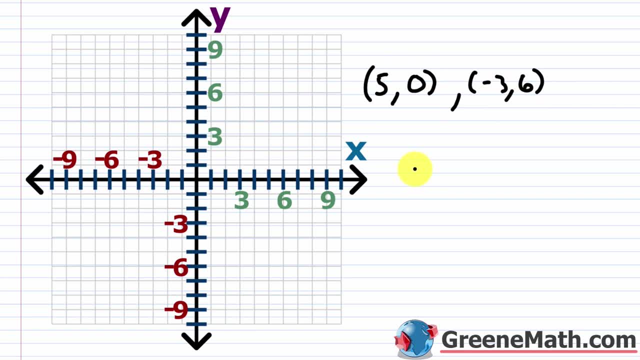 negative 3 comma 6.. So if we want to plot these, let's go to 5 comma 0 first. So that guy, we're just going to go 5 units to the right, We're not going to move it all vertically. So this is 5. 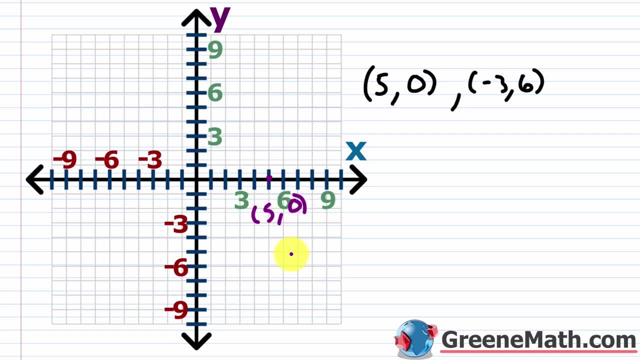 comma 0. So let me label that This is 5 comma 0 and negative 3 comma 6.. So I'm going to go 3 units to the left and 6 units up. That's going to be right there. So I'm going to call this negative. 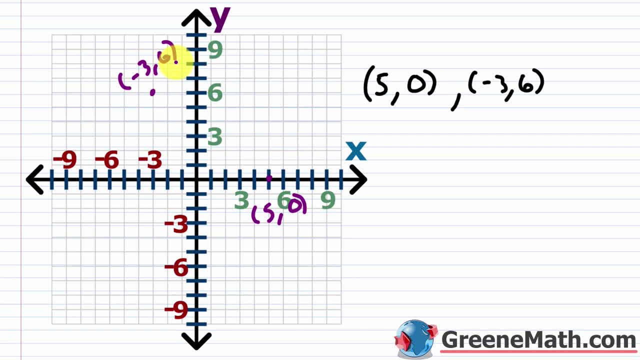 3, comma 6.. So let me draw a line connecting the points. So this line right here that represents the distance between the two points will be c, or the hypotenuse. Now what I'm going to do to make a right triangle, I'm going to take an x value from one of the points and I'm going to take a. 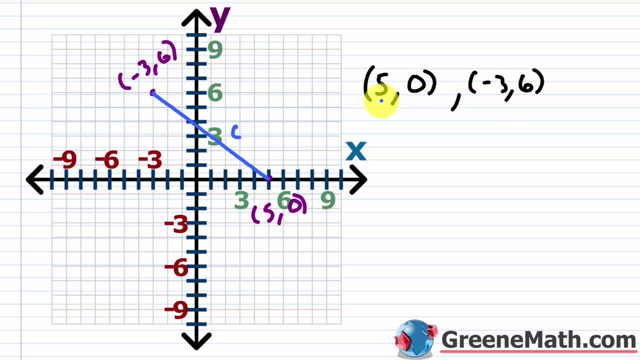 y value from the other. So in other words, I could take 5 from this guy and 6 from this guy, So I could make a point 5 comma 6. That would complete my right triangle. So if I go to 5 and then up to, 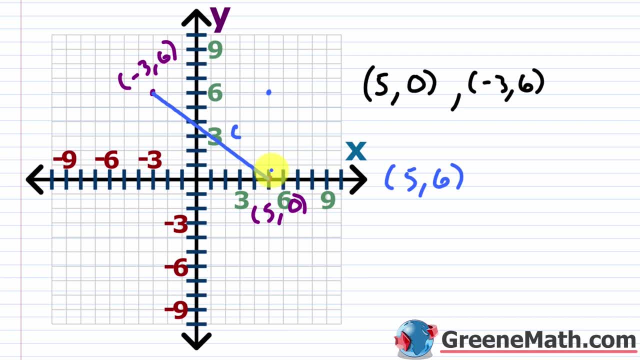 6, so that right there would give me a right triangle. Now I'm not going to do it that way because I can do it another way and it's going to be easier for us. So I'm going to take an x value of negative 3 and a y value of 0. So I'm going to go to negative 3. 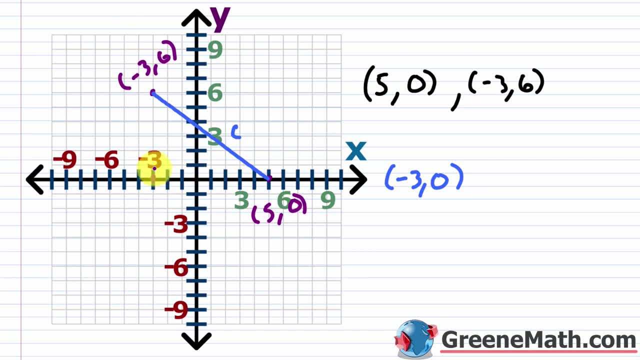 comma 0 on the number line. It's going to be right here. So that's another way you can kind of complete that guy. So take an x value from one point and a y value from the other. That's how you can get your kind of third vertex for the right triangle. So let's kind of fill this in now. 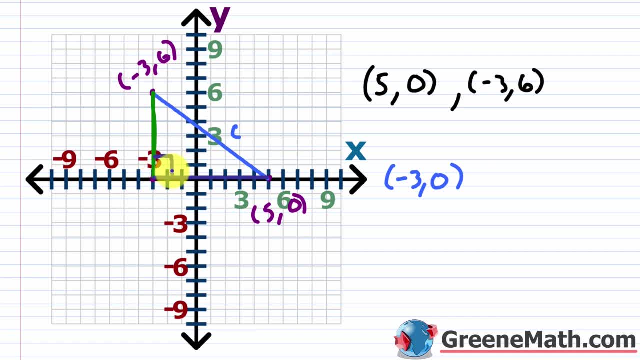 Okay, so not perfect, but you get the idea. Let me draw this symbol here real quick. So we have a 90 degree angle, Okay, so I'm just going to go ahead and label this kind of horizontal measure from here to here. I'm going to label that as b and I'm going to label this: 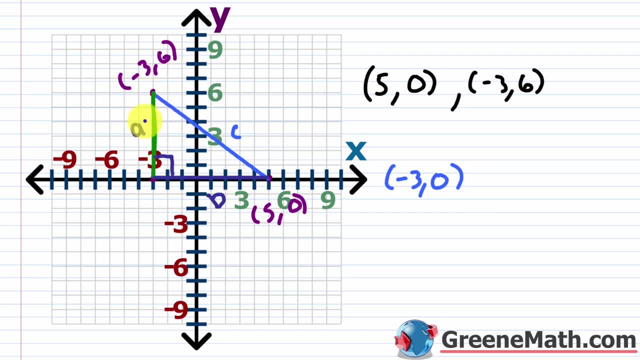 vertical measure from here to here. I'm going to label that as a. Okay, so how can we find the measure for b and the measure for a? We know that we're going to end up solving for c, but b and a should be easy to find. So for b, what do I want? This is a horizontal line, So 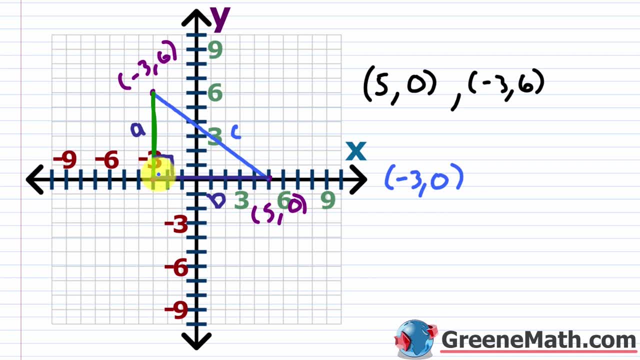 think about the x axis or the x values. What is the x value here and what is the x value here? Well, let me kind of write this point in here: This is negative three, comma zero. So the x value here is negative three and the x value here is five. So just think about this before we kind of 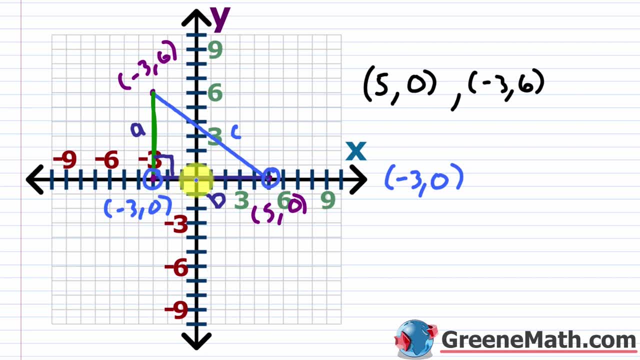 do any procedure. Just think about this: If I go from negative three to zero, I've traveled three units, And then if I go from zero to five, I've traveled another five units. So three plus five is eight. So that tells me the distance or the measure for b is going to be eight, But we're 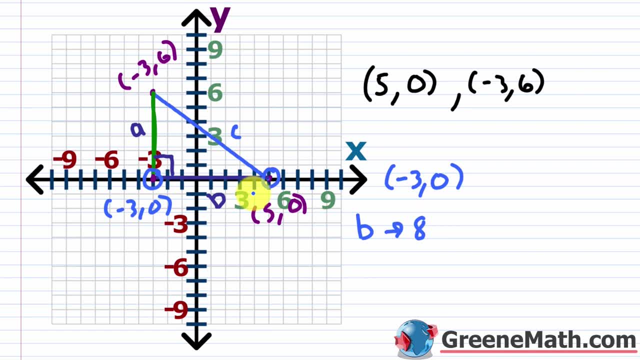 not going to pull out a coordinate plane each time and count things. We need a better procedure. So, basically, if I'm looking at the x value here, I'm going to be able to do this. I'm going to be at this distance here. I want the difference in x values. But because we want to guard against, 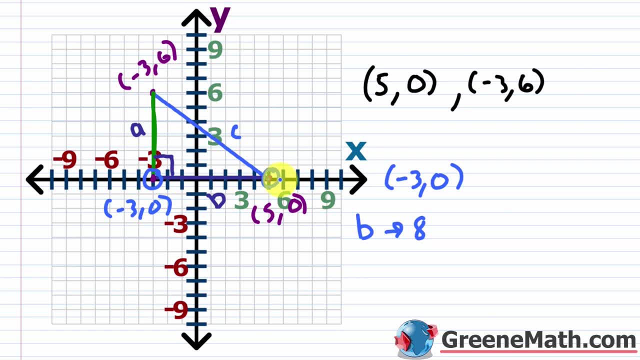 getting a negative answer right, because we don't want a negative distance. we can do this inside of absolute value bars. So I could say that I have the absolute value of negative three, which is the x coordinate here, minus five, which is the x coordinate there. This is equal to the 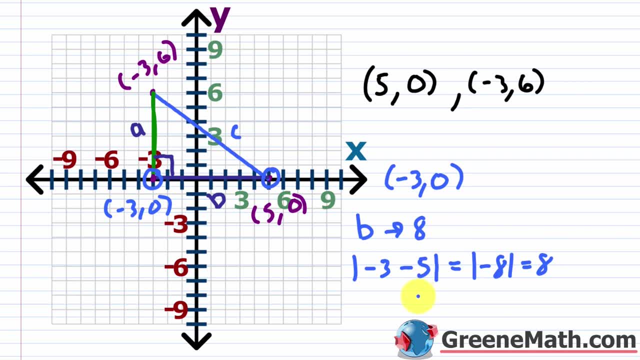 absolute value of negative eight, which is equal to eight, which is what I got. Or you could also do it the other way. Okay, the order isn't going to matter. So you can go ahead and say that you have five minus a negative three, which is five plus three, So the absolute value of that. 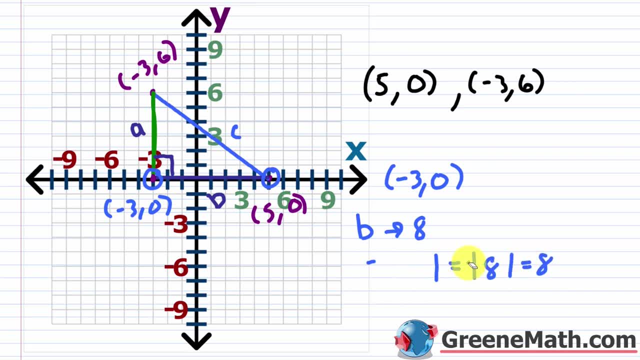 would be the absolute value of eight, which is also eight, Okay. Now, similarly, when we look at, kind of the measure of a, now I'm looking at a vertical line. So with a vertical line, I'm thinking about y values. okay, because you're thinking about this as being parallel to the y. 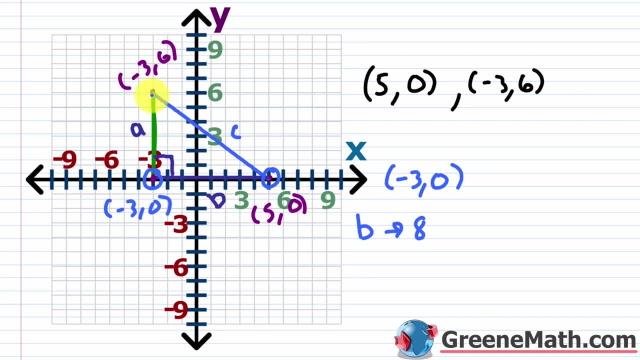 axis. the y axis is going up and down. Okay, so now we're thinking about y values. So here I have a six for a y value And here I have a zero. Okay, so for those two points again from here. 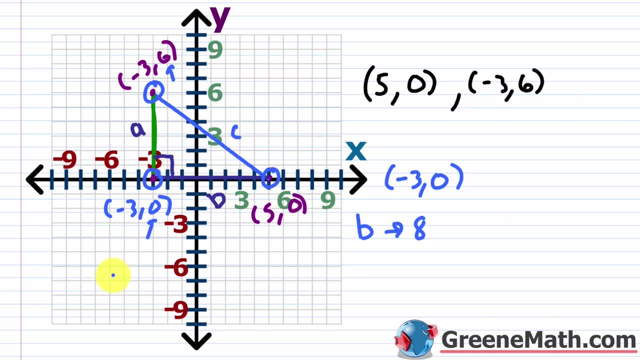 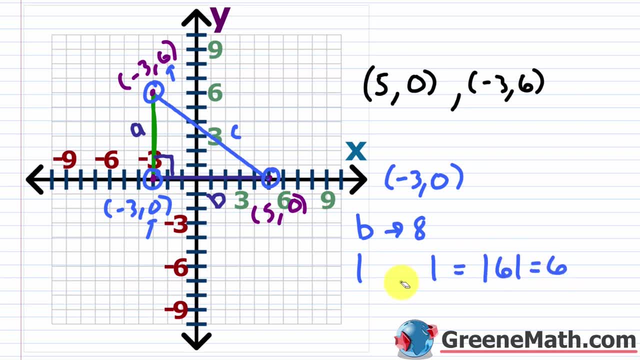 absolute value of six, which is six. or I could flip that around and say the absolute value of zero minus six, which is the absolute value of negative six, which is also six. Again, the absolute value operation is just there to make sure that we don't get a negative distance. 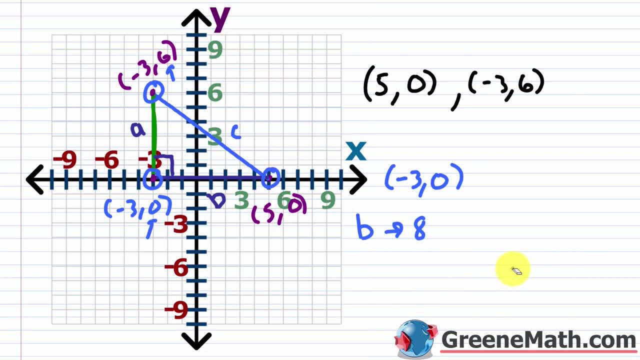 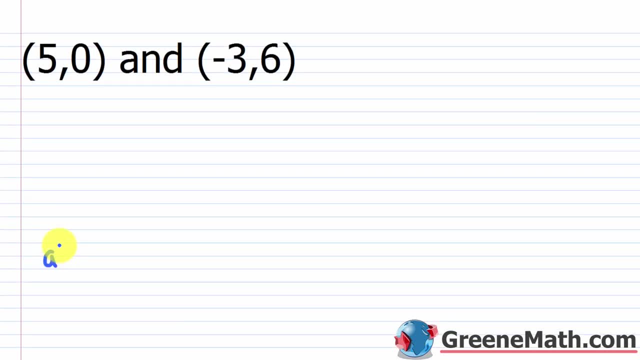 Okay. So once we have the value for B and A, we know that we can solve for C. So let's go to a different page. So again, I'm just going to write that A squared plus B squared equals C squared. So for A, we know that this guy was six. For B, we know this guy was eight. So if I plug in there, 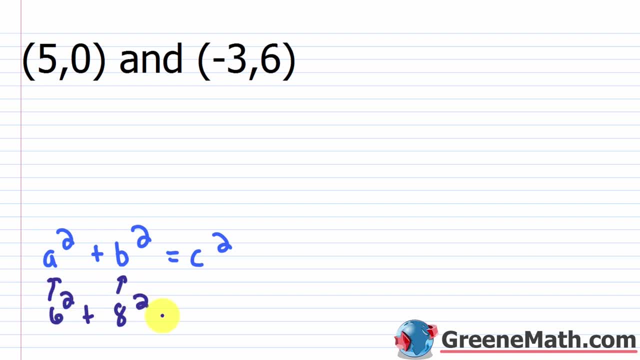 what's going to happen is I'm going to have six squared plus eight squared is equal to C squared. Let me kind of move this up a little bit And I'll erase this. We don't need this anymore. Kind of write that in: So six squared is 30.. 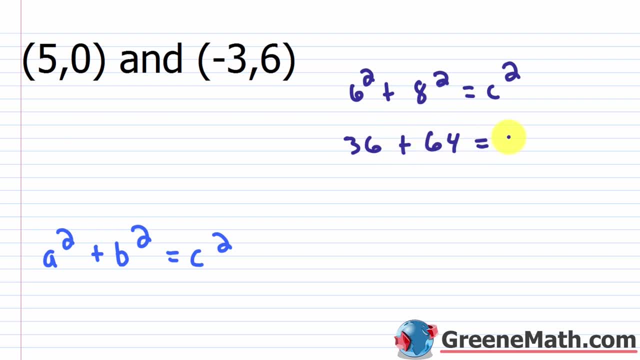 Six plus eight squared is 64. This equals C squared. 36 plus 64 is 100. So you get 100 is equal to C squared. Now we would take the square root of each side to get C by itself. So you take square root of this side. You're used to doing this. You'll say plus or minus. 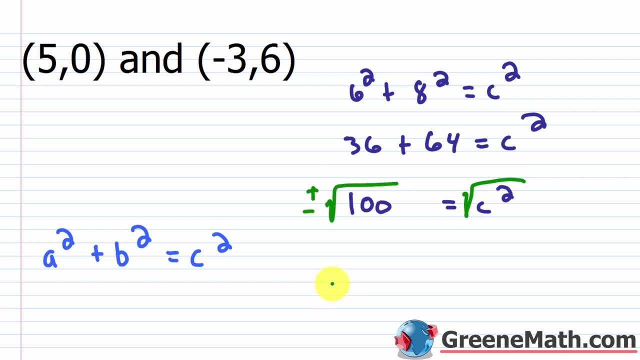 the square root of this side. So what you're going to see in a minute is one of these solutions you can throw up, So you'll have: plus or minus. 10 is equal to C. So basically, C is going to be equal to plus or minus 10.. 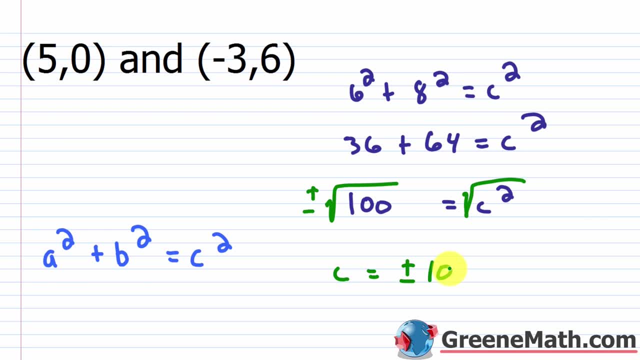 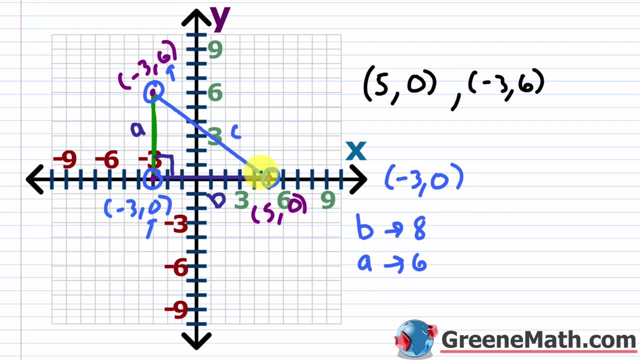 Now, does it make sense for C to be equal to negative 10?? If I go back, does it make sense for the distance from here to here to be negative 10?? No, because the distance can't be negative. So when we do this guy, we just need the principal square root, right. We don't need to think about. 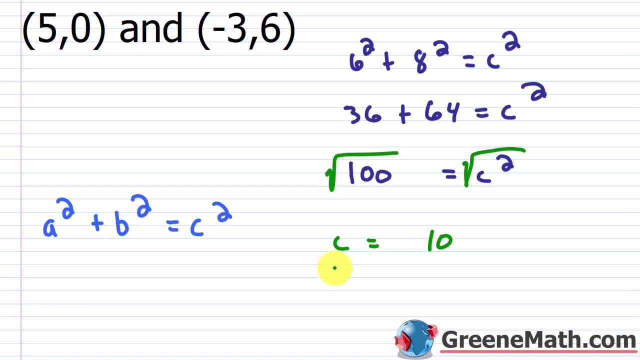 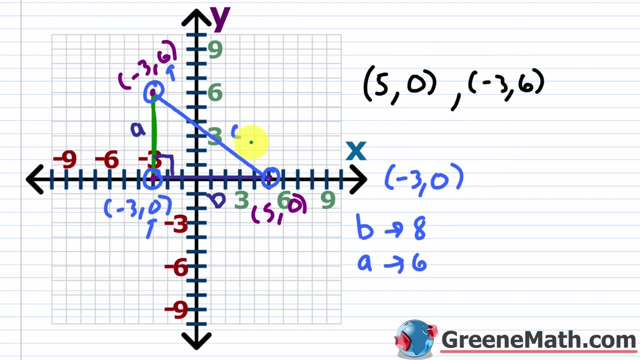 any negatives there, because that would basically be nonsense, right? So C: there the distance between these two points is going to be 10.. So that's going to be my distance. So if I go back this guy right here, if I wanted to label it, I could say this is 10.. We already know that B is 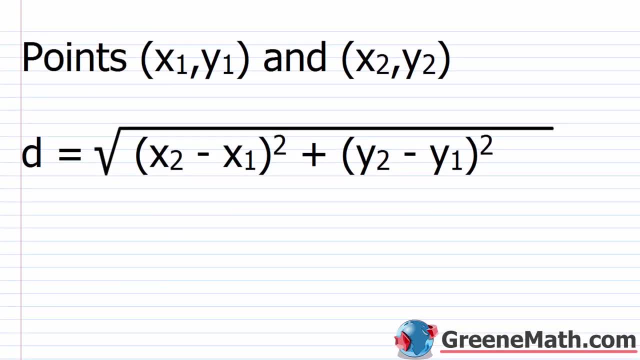 8, and we know that A is 6.. So now that we've seen an example of this on the coordinate plane, let's make it very, very simple. So all you really need is this formula here, and I'll kind of 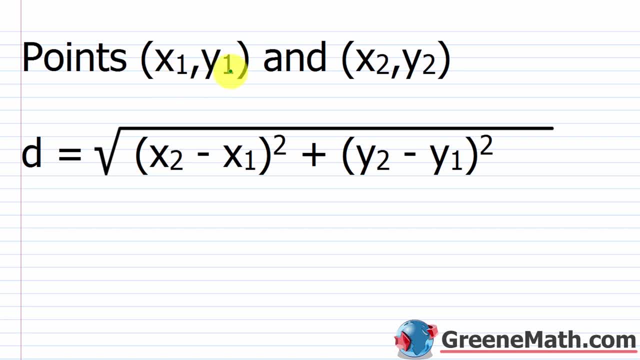 explain where this comes from. So if you have points x sub 1, y sub 1, and x sub 2, y sub 2, you just plug into this formula and you'll find the distance between the two. So let's say we go. 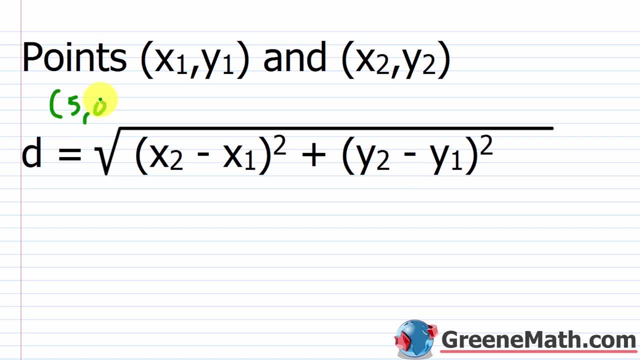 with our original example. So we had 5, 0, and we had negative 3, 6,, right? Those were our two points. So let's label this first. Let me kind of drag this over here, so it's not in the way. Let's label this first one as x sub 1,. 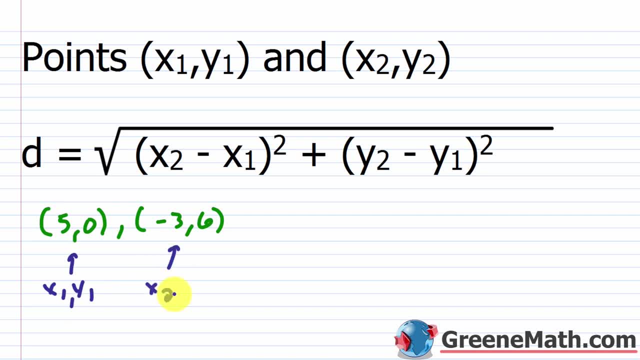 y sub 1.. Let's label this second one as x sub 2, y sub 2.. And again, it doesn't matter which one you label as which. okay, You can plug in whichever one you want for either. So my distance is going. 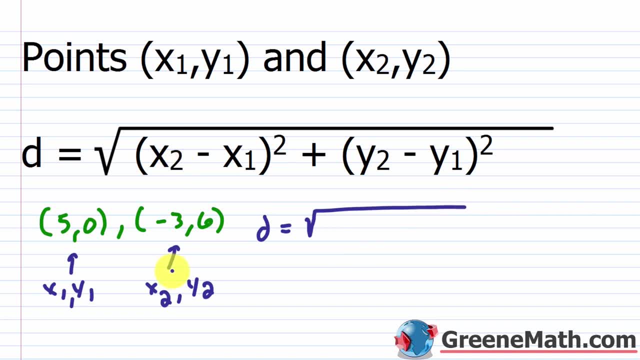 to be equal to the square root of. so you have your x sub 2,, which in this case is negative, 3, minus your x sub 1, which is 5.. This quantity is squared, Then plus, you're going to have: 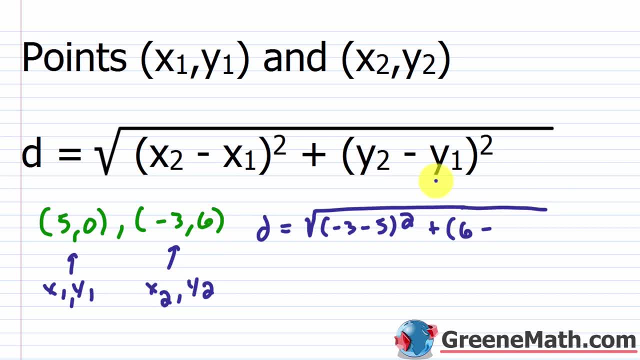 your y sub 2,, which is going to be 6, and you're going to have your y sub 2,, which is going to be 6,, minus your y sub 1,, which is going to be 0,. this quantity is squared. Now, before we do, 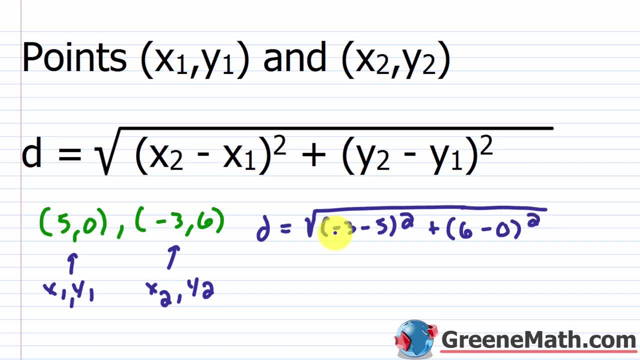 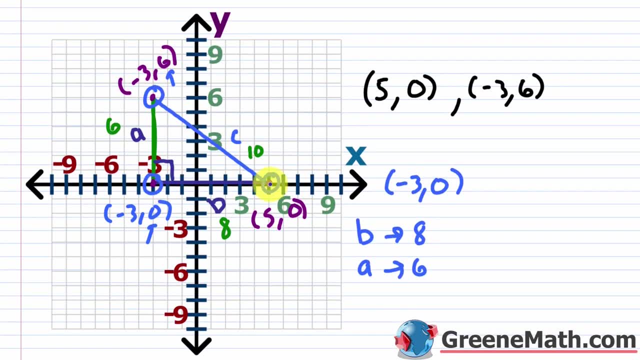 anything. I want you to remember where we got this from. This negative 3 minus 5 was what. This was the horizontal distance if we go back from right here. right, It was the difference in x values. So that's all we need to do. We take the difference in x values Now. in this case, we did it in. 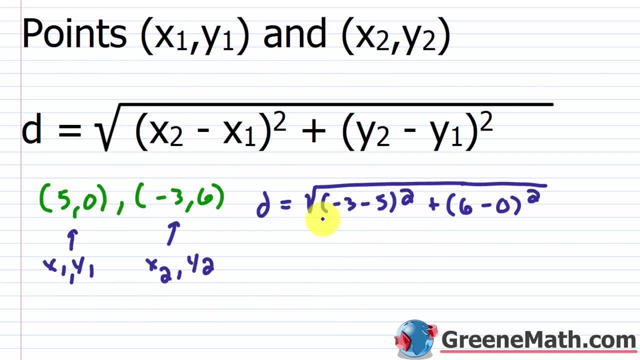 absolute value bars. but when we come here, we don't see absolute value bars. That's because we're squaring the result, okay. So if this was negative when we square it, it becomes positive. If it was positive when we square it, it stays positive. okay, So that's why you don't need 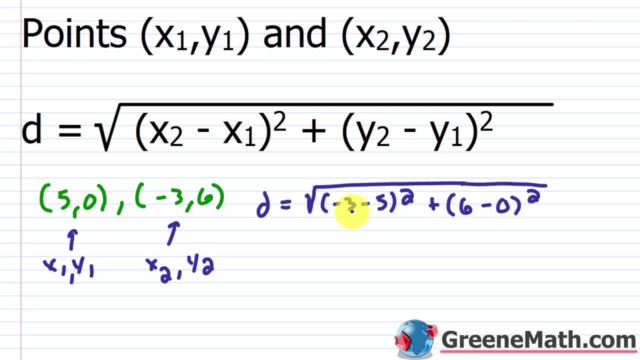 absolute value bars there. So negative 3 minus 5 is negative 8.. Negative 8 squared is 64. So this is 64 here. Then here we have the difference in y values, So 6 minus 0.. So if we 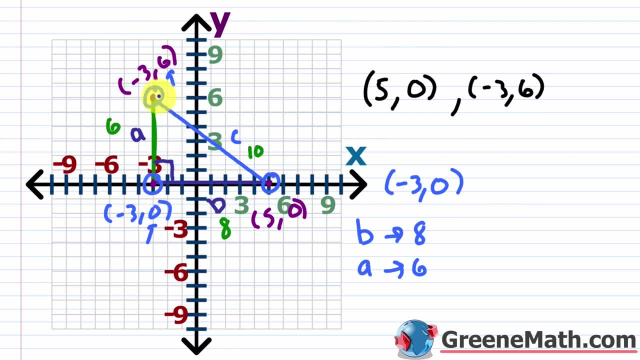 go back up again. that's the same thing we did here. We had a y coordinate of 6.. We had a y coordinate of 0. We take the difference between the two Again, when you do it on this, you take. 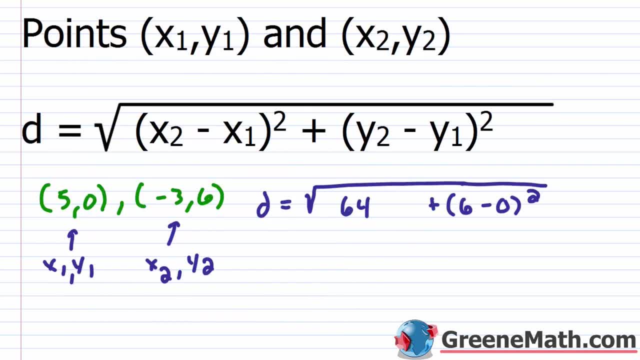 the absolute value bars. So you don't need absolute value bars there. So you don't need absolute value, right? But when you get to the formula, you don't need the absolute value operation because again you're squaring it. okay. So 6 minus 0 is 6.. 6 squared is 36.. 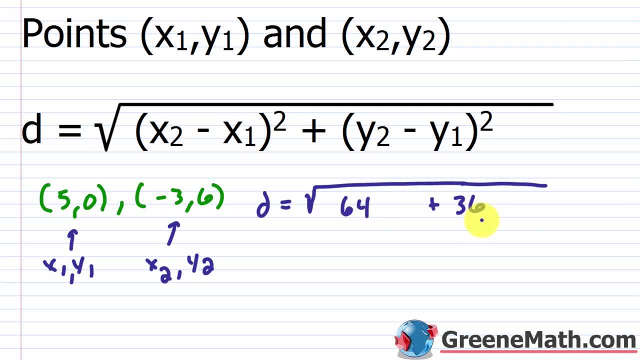 So at this point we have what We have, our a squared plus our b squared, And essentially, if I erase this, I could say that d squared, which just took the place of c squared, we just relabeled it as d for distance, okay, So that's clear. We'll just kind of change this back So. 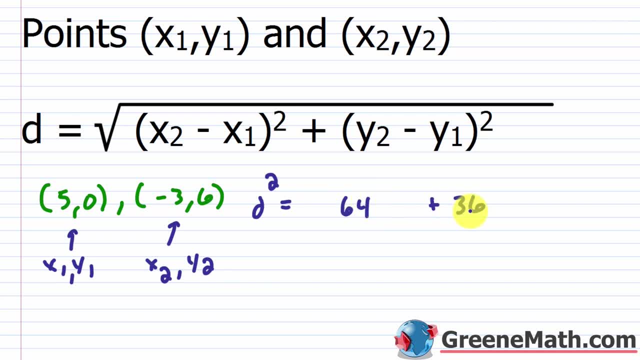 d squared is equal to. this was our b squared plus our a squared. Well, what happens is to get d by itself. I just take the principal square root of each side right. I don't need to go plus or minus, because the negative solution will be thrown. 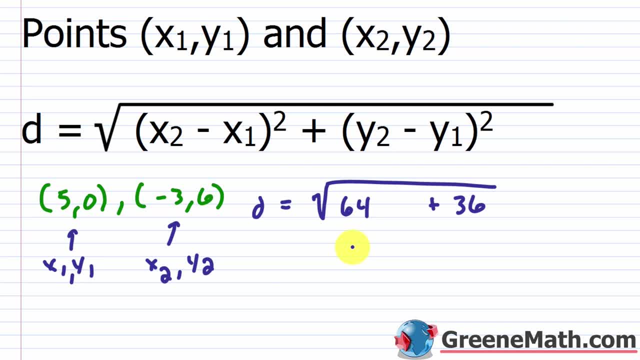 out. You don't want a negative distance. So at this point we pretty much just solved. So 64 plus 36 is 100.. And then the square root of 100 is 10.. So d equals 10.. So much much quicker to just use. 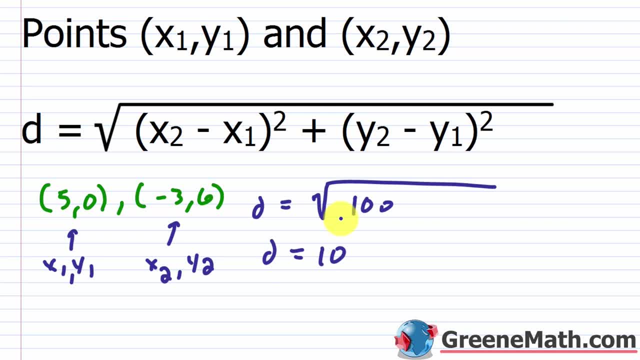 the formula, But I want you to understand where it comes from so that in a pinch, if you can't remember it, you can go back through and say, okay, well, if I had, you know, a squared plus b squared equals c squared. okay, well, I know that one of these is going to be the difference. 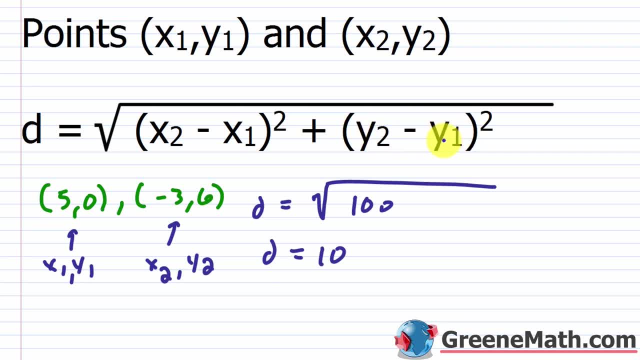 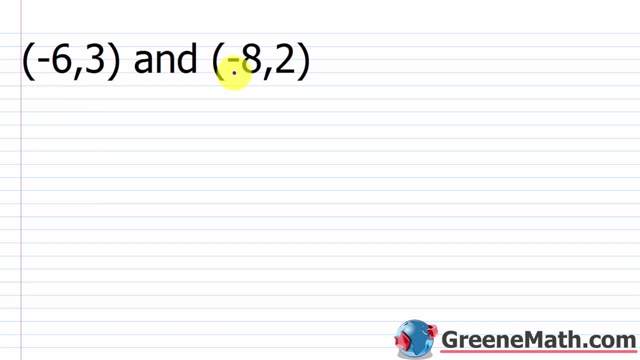 in x values. one of these is going to be the difference in y values. you know, so, on and so forth. you can derive the formula. All right, let's take a look at another example. So we have negative 6 comma 3 and negative 8 comma 2.. So let's just label this as x sub 1, y sub 1.. Let's 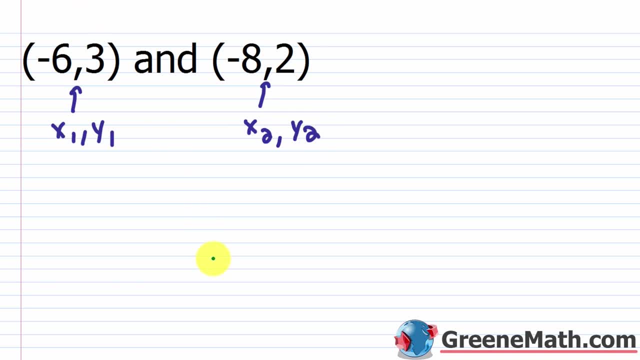 label this as x sub 2, y sub 2.. And what I'm going to do is just plug into the distance formula. So d is equal to the square root of, so you have your x sub 2 minus your x sub 2, minus your x sub 2,. 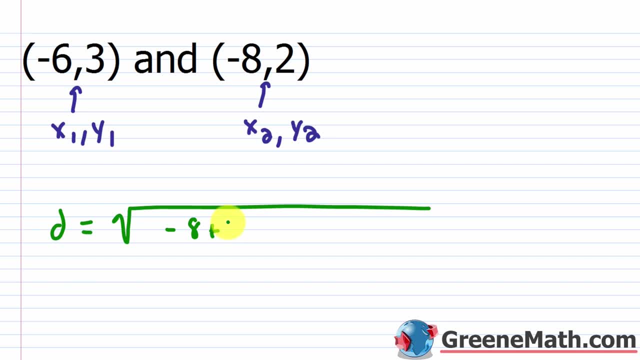 so negative 8 minus a negative 6, so that's plus 6, to make that better. And this is wrapped inside of parentheses and squared, and plus your y sub 2,, which is 2,, minus your y sub 1,, which is 3,. 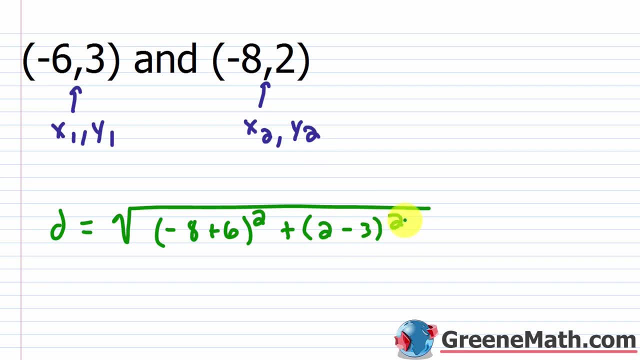 again wrapped inside of parentheses and squared. So negative 8 plus 6 is negative 2, negative 2 squared is 4.. So this is 4.. 2 minus 3 is negative 1, negative 1 squared is 1.. So this is 4 plus 1. 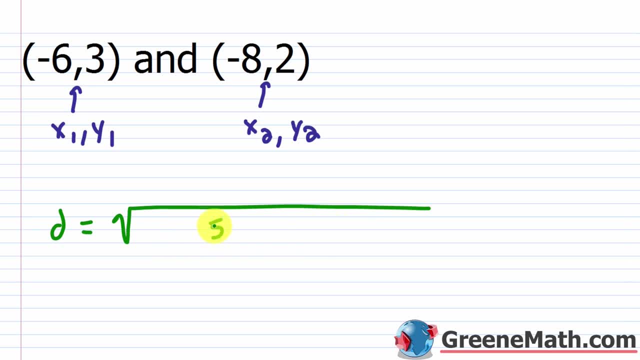 or 5.. So the distance between the two is going to be the square root of 5, okay, So the distance is the square root of 5.. Let me make that a little bit better. And this, basically, is an irrational number. So to get an exact value, you'd leave it in this form If you wanted to. 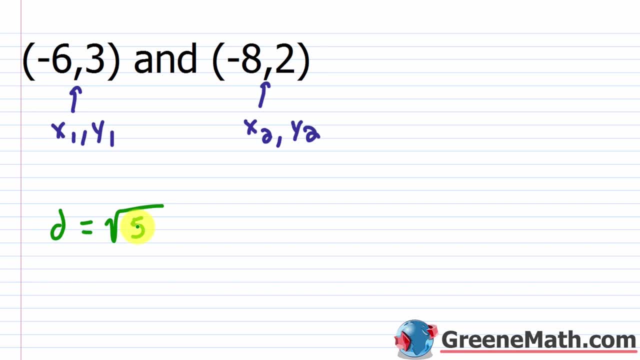 approximate it. you could punch it up on a calculator and you'd get about 2.24,. okay, if you wanted to approximate it. But again, if you want an exact value, go with just square root of 5.. All right, let's take a look at another one. So we have negative 2 comma 4 and negative 4 comma. 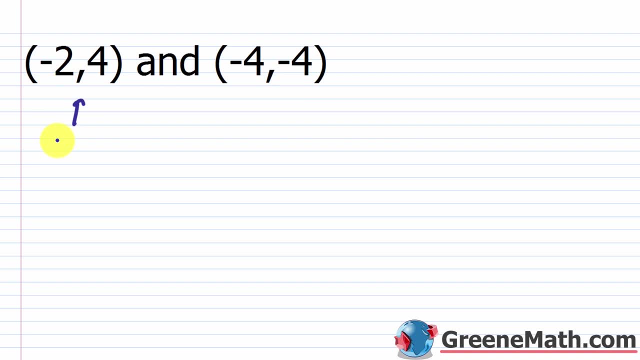 4.. I'm just going to change the order up and I'm going to say this first point is x sub 2, y sub 2.. And I'll say the second point is x sub 1, y sub 1, okay, So I'm going to plug into my distance formula So the distance is. 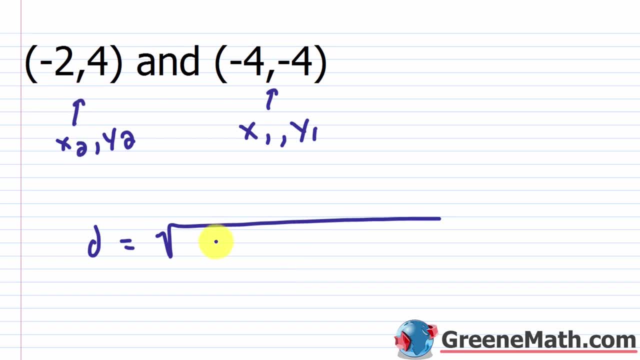 equal to the square root of. So for the formula, you have x sub 2,, which is negative, 2, minus x sub 1,, which is negative 4.. So minus a negative is plus a positive. So negative 2 plus 4.. This is. 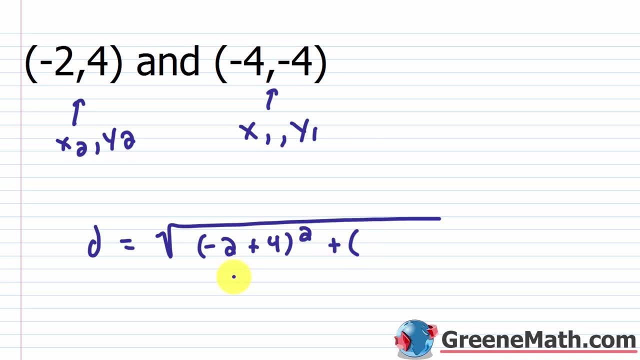 wrapped in parentheses and squared, Then plus, we're going to have our y sub 2,, which is 4, minus our y sub 1, which is negative 4.. So minus a negative is plus a positive. Again, this is wrapped in parentheses and squared. So negative 2 plus 4,. 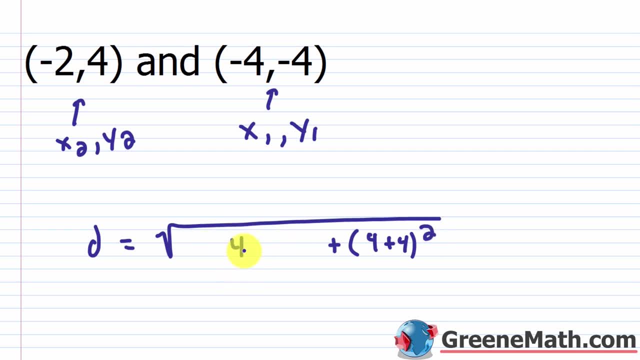 is 2.. 2 squared is 4.. So this is 4.. 4 plus 4 is 8.. 8 squared is 64.. So if we take the sum of these two values, 4 plus 64 is going to be 68. So this is going to end up being the square root of 68.. 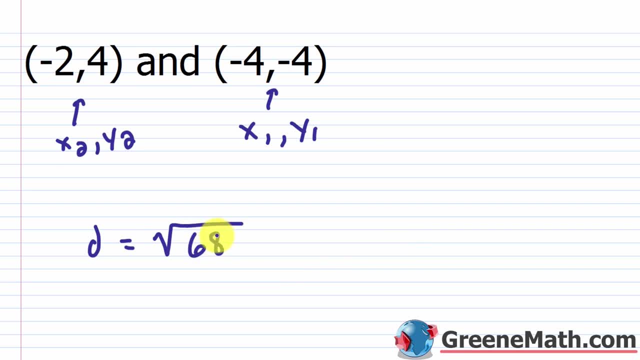 Now you can simplify this, because 68 factors in a 4 times 17.. So what I could say is that this is the square root of 4 times 17.. Square root of 4 is 2.. So I can say this is 2 times. 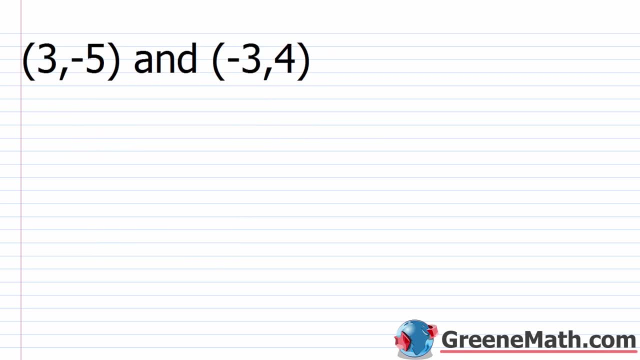 the square root of 4 times 17.. So I can say this is 2 times the square root of 4 times 17.. All right, let's take a look at one more. So we have the distance between these two points. We. 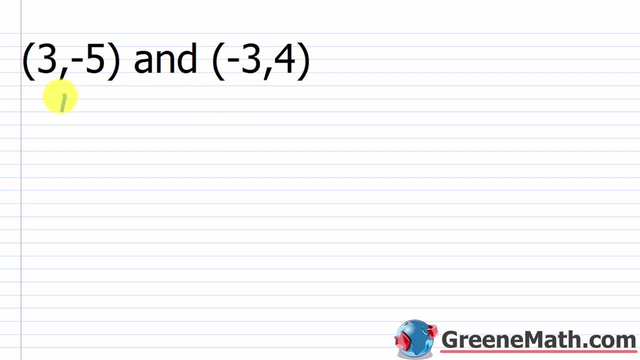 have 3 comma, negative 5 and negative 3 comma 4.. So let's label this first point as x sub 1, y sub 1.. Let's label this second point as x sub 2, y sub 2.. So the distance between the two 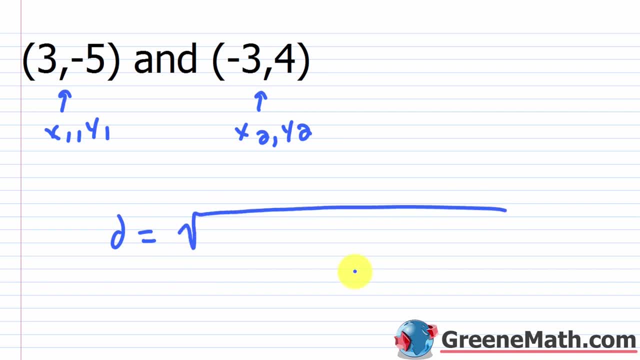 again, the distance is equal to the square root of. you've got x sub 2,, which is negative, 3, minus x sub 1,, which is 3.. Okay, that's wrapped in parentheses and squared. Then plus, you've got your y sub 2,, which is 4,, minus your y sub 1,, which is 4,. 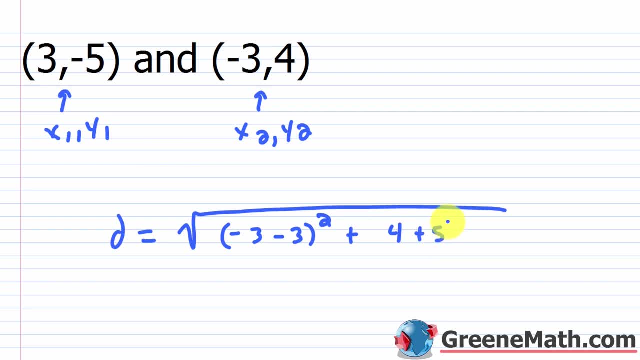 minus your y sub 1.. So minus a negative 5 would be plus 5.. Again, this is wrapped in parentheses and squared. So negative 3 minus 3 is negative 6.. Negative 6 squared is 36.. So this is 36.. 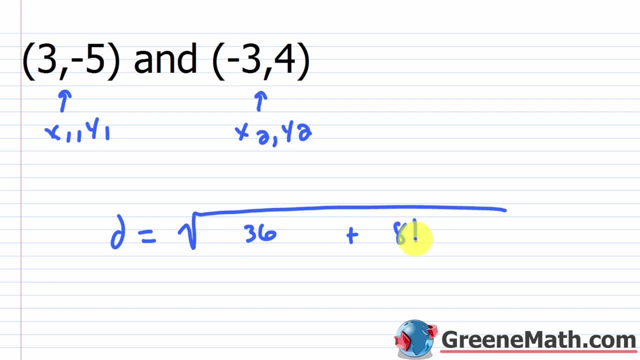 And then 4 plus 5 is 9.. 9 squared is 81.. So 36 plus 81 is 117.. So this would be the square root of 117.. This can be simplified: 1 plus 1 is 2.. 2 plus 7 is 9.. So we know. this guy is divisible by: 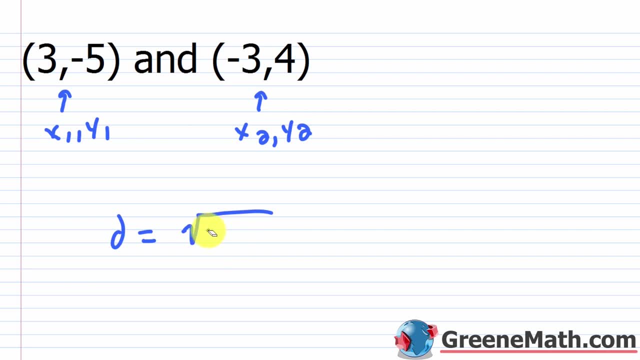 9.. It's going to end up being 13 times 9.. So 13 times 9, square root of 9 is 3.. So I can go ahead and write this as 3 times the square root of 13 as my answer. Hello and welcome to Algebra 2, Lesson 57.. 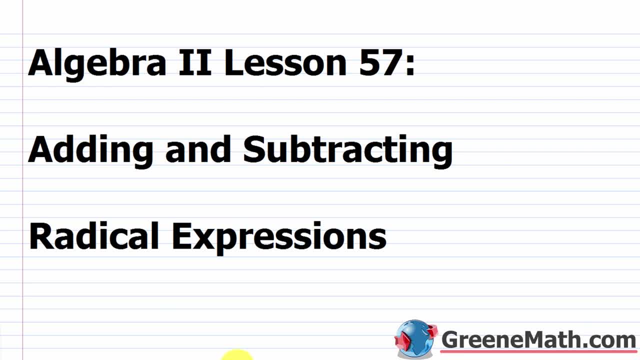 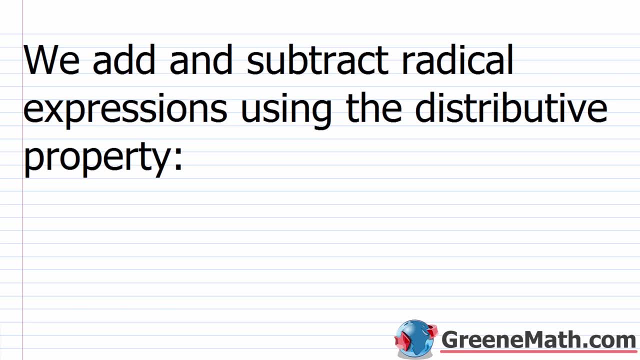 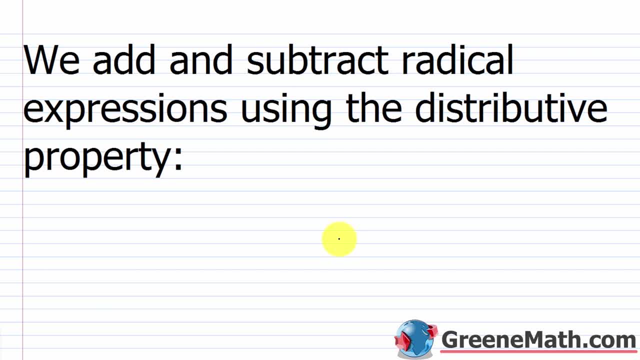 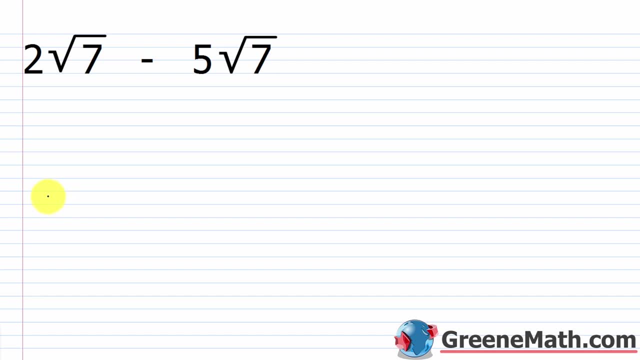 by talking about this topic of adding and subtracting radical expressions. So we have here that we add and subtract radical expressions using the distributive property. So this is something similar to when we combined like terms. So, for example, if we had something like, let's say, 2x. 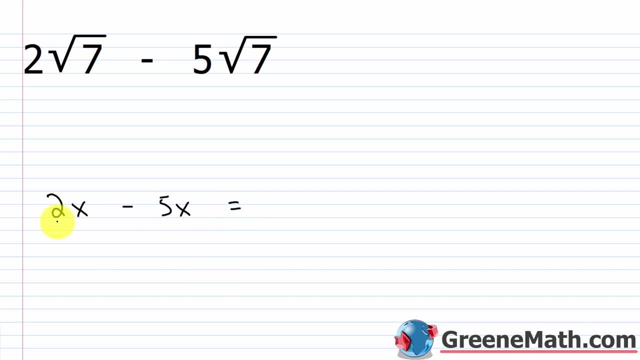 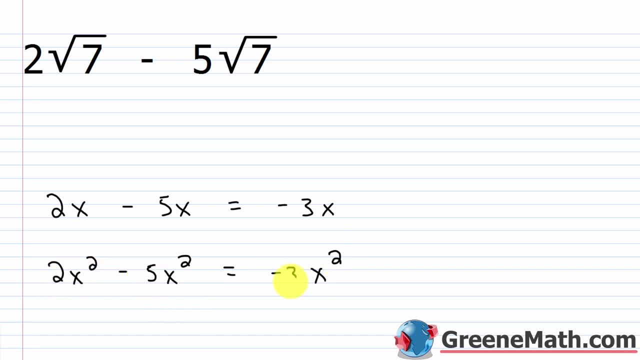 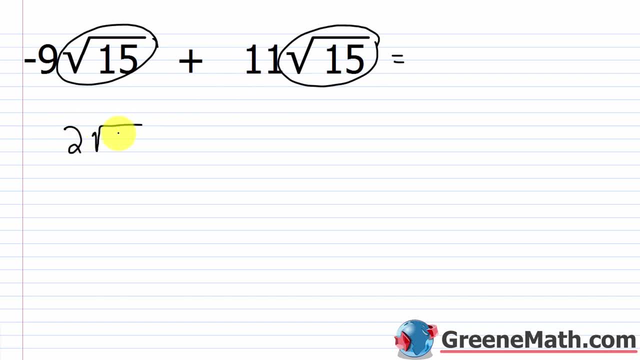 then times that common value of 2 minus 5 is negative 3.. And and then times that common radical the square root of 15.. Now, as I alluded to, for this to work we've got to have like radicals. 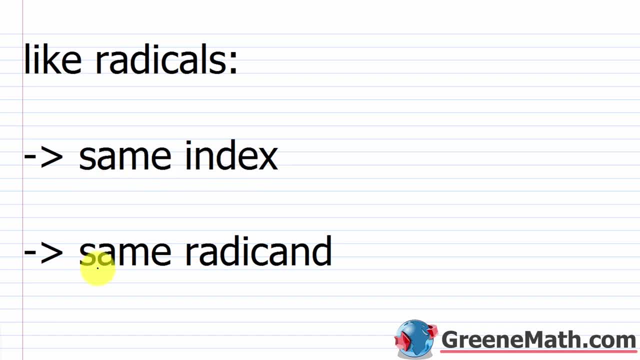 Like radicals, have the same index and the same radicand. Now again, we talked about something similar to this when we were working with polynomials. Remember we had like terms, same variable raised to the same polynomial. Well, for, like radicals, it's the same index with the same radicand. 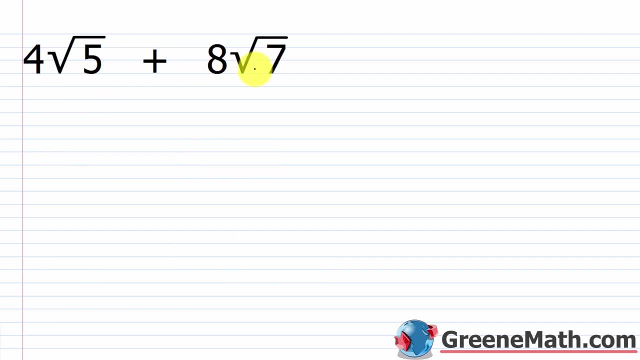 So let's say we see something like this: 4 times square root of 5 plus 8 times square root of 7.. Can I do the same technique to simplify here? No, I cannot. I have a square root in each case, so the index is the same. 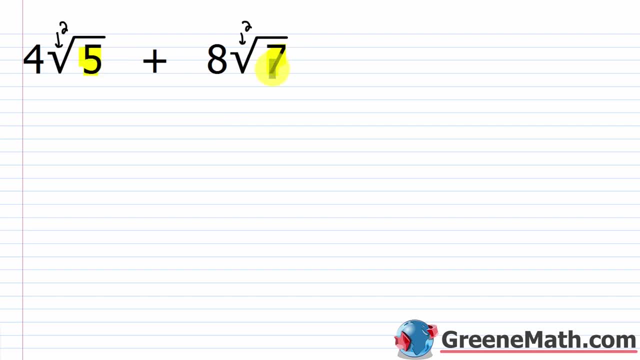 But my radicand here is a 5,, my radicand here is a 7.. So these are not like radicals, right? So not like radicals here. And it's the same thing as when we saw something like, you know, 4x squared plus 5x. 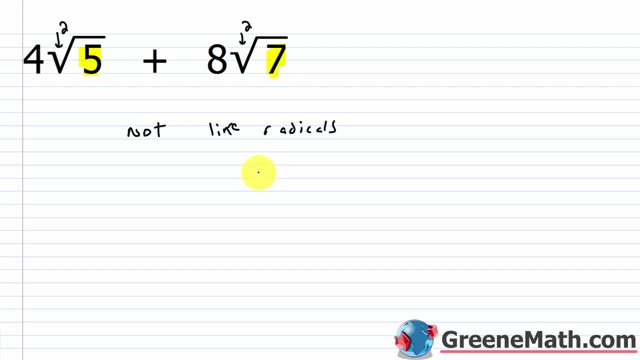 5x cubed. Those are not like terms so we can't do anything to simplify there. All right, here's another example. So we have negative 3 times the cube root of 7, minus 2 times the fourth root of 7.. 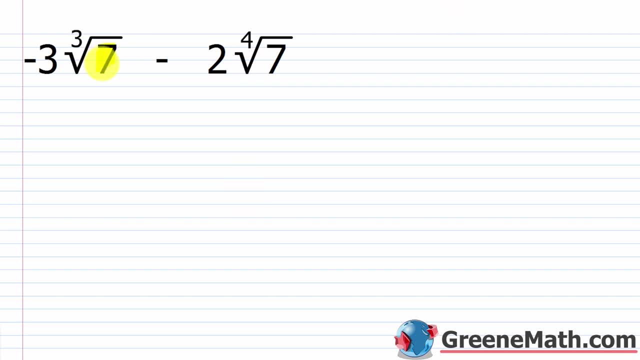 So in this case the radicand is the same, So you've got a 7 here and a 7 here, But the indexes are different. This is a 3, right, It's a cube root. This is a fourth root. 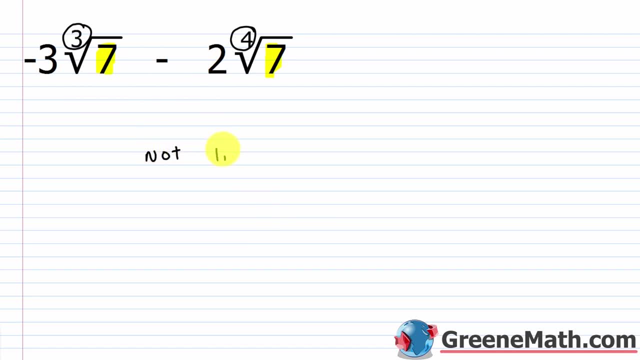 So these are not like radicals. So these are not like radicals. And again, this is the same thing as when we came across non-like terms when we were working with polynomials, So we're not going to simplify this any further than that. 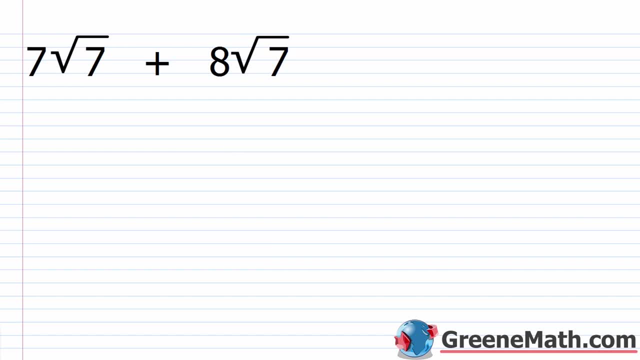 All right, let's look at some problems where we can do some simplifying, And we'll come across some things where we have to simplify before we can do addition or subtraction. So we have 7 times the square root of 7 plus 8 times the square root of 7.. 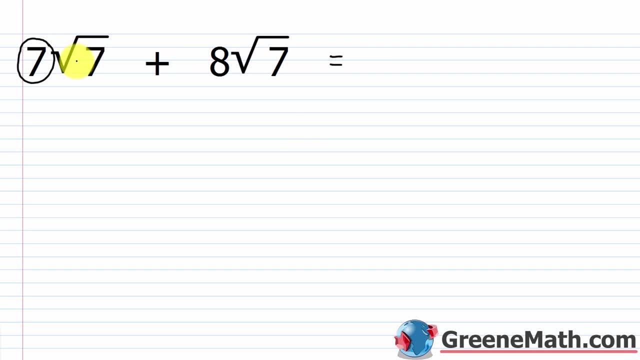 So again, all I need to do is look at the numbers that are multiplying the radicals. So we have 7 plus 8.. That's 15 times that common radical. That's the square root of 7.. All right, what about negative, 8 times the square root of 10 plus 5 times the square root of 10?? 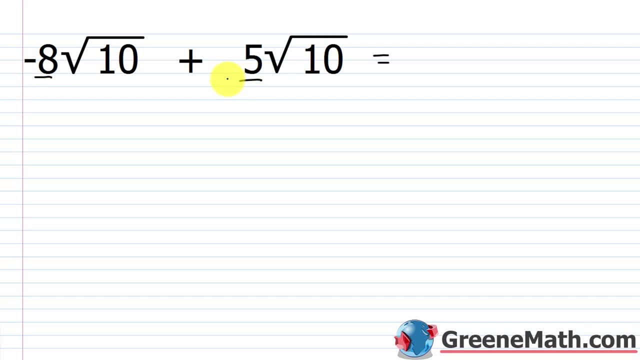 Again, all I'm looking at is negative 8 and 5.. So negative 8 plus 5 is negative 3. And then times the square root of 10.. All right, now we have 2 times the square root of 24 minus 8 times the square root of 24.. 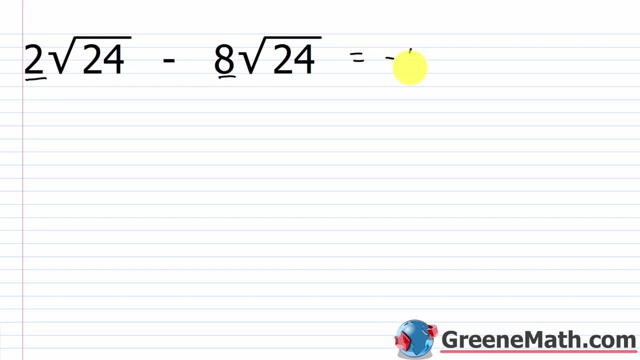 So 2 minus 8 would give me negative 6. And then times the square root of 24.. Now you don't want to remember, You don't want to report your answer in this format. because why? The reason is, if you look at the square root of 24, this is not simplified. 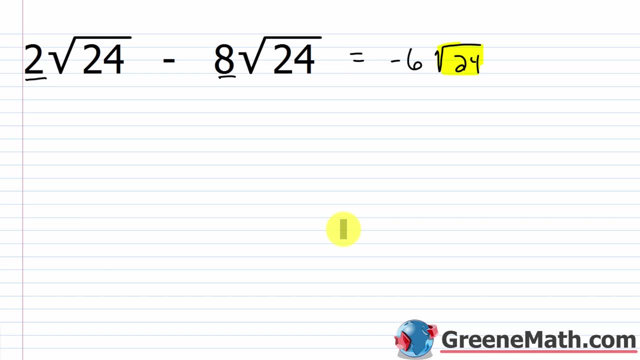 We know that if we factor 24, we could get a perfect square from 4.. 24 you could make as 4 times 6.. 4 is a perfect square, So we want to simplify this. So let's make this negative: 6 times square root of 4 times square root of 6.. 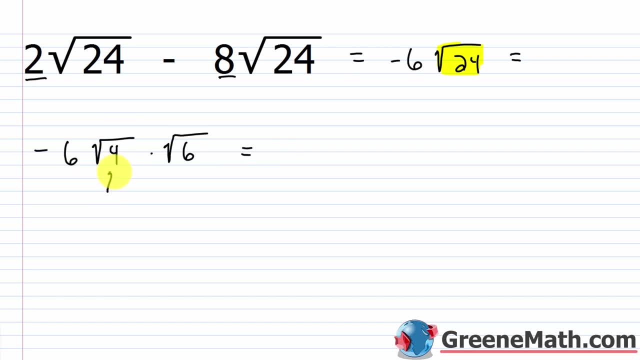 This would give us negative 6 times The square root of 4.. So I could replace that with a 2.. Negative 6 times 2 would give me negative 12.. And then times the square root of 6.. Now this is simplified because the square root of 6, I can't do anything else with that. 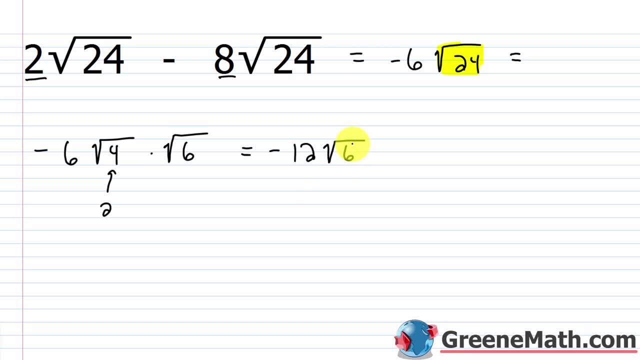 6 factors into 3 times 2.. No perfect squares in there, So we're basically good to go All right. for the next one, we have 2 times square root of 20, minus 3 times square root of 5, plus 2 times square root of 5.. 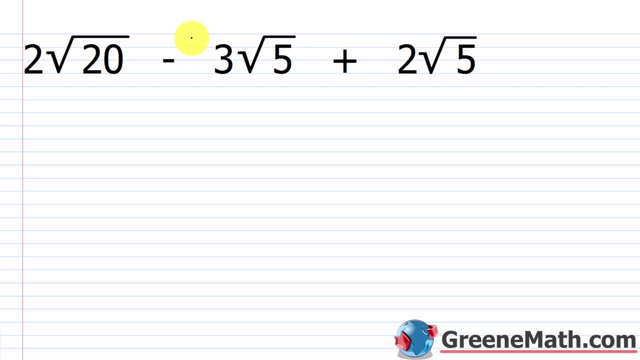 So you might look at this and say, well, you've got the same index in each case, but I have a 5.. A 5 is a radicand here and a 5 is a radicand here, but a 20 as the radicand here. 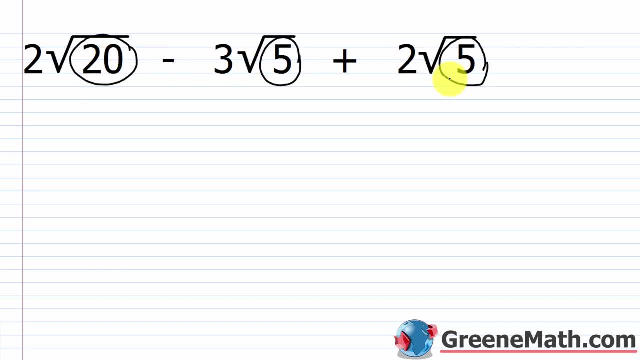 So I can't combine this with any of these. Before you do that, make sure that you factor things, Because if I look at 20, we know it's what It's: 5 times 4.. 4 is a perfect square, so that can come out. 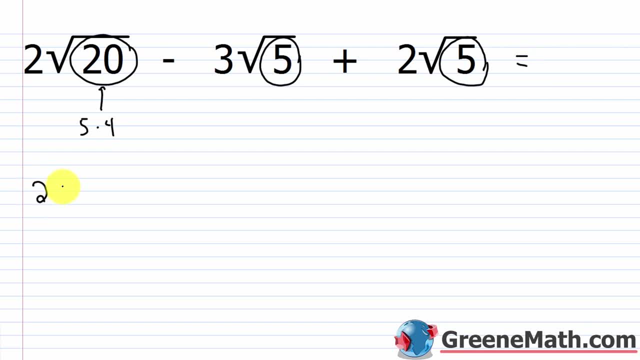 So, really, what I can do is I can say: this is 2 times the square root of 5, times the square root of 4.. Minus 3 times the square root of 5, plus 2 times the square root of 5.. 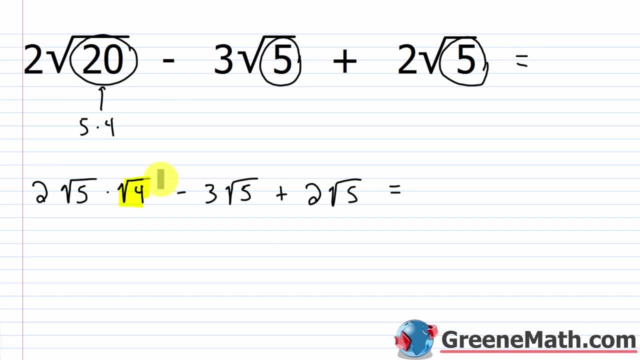 This is equal to. We know that the square root of 4 is 2.. So if this is 2, you'd have 2 times 2, which is 4 times the square root of 5 minus 3 times the square root of 5 plus 2 times the square root of 5.. 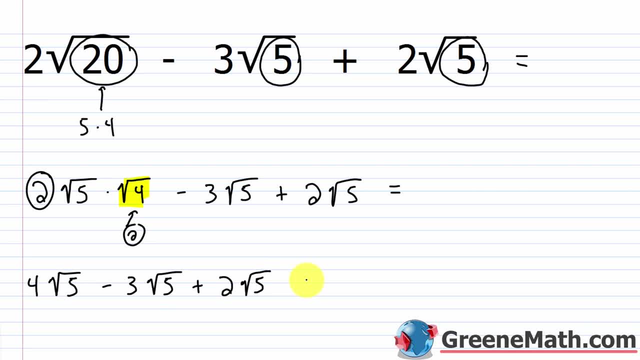 Now that we've simplified these are all like radicals, so I can just work with the numbers out in front. So in other words, I would say 4. minus 3 is 1.. 1 plus 2 is 3.. 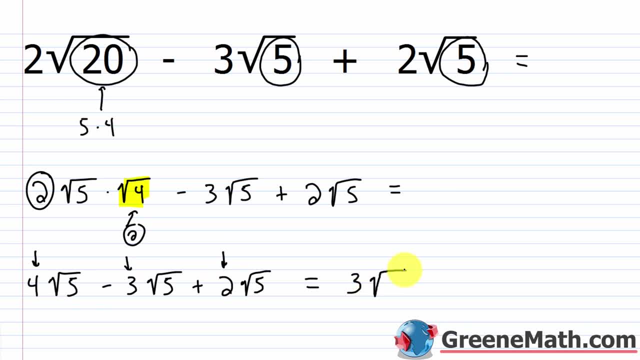 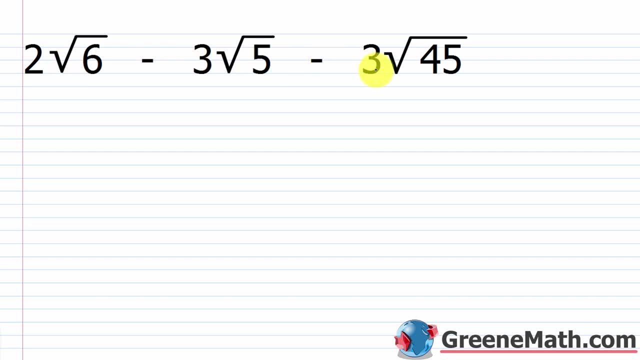 So this would be 3 times that common radical, which is the square root of 5.. Alright, what about something like this: We have 2 times the square root of 6, minus 3 times the square root of 5, minus 3 times the square root of 45.. 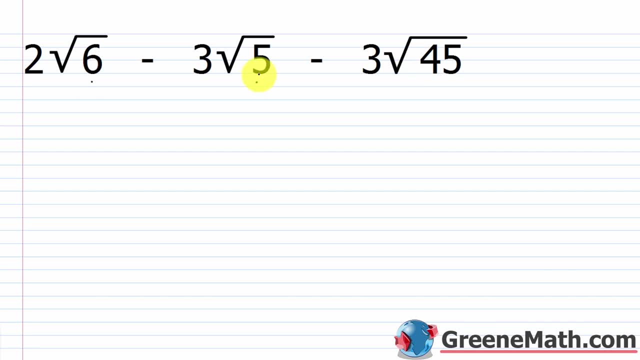 Now square root of 6- I can't simplify any further. Square root of 5- I can't simplify any further- But square root of 45, we can do something with that, For the square root of 45, 45 is. 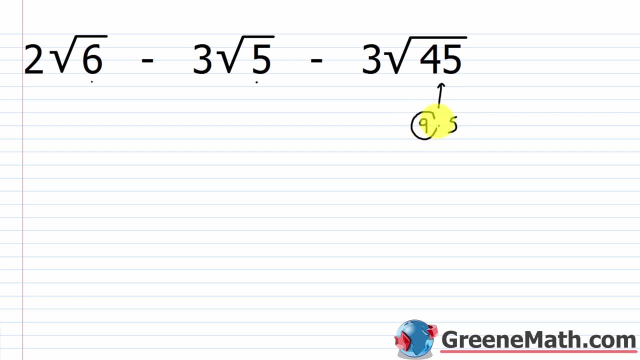 9 times 5.. 9 is a perfect square, So what I can do, we can write: 2 times the square root of 6, minus 3 times the square root of 5, minus 3 times the square root of 9. 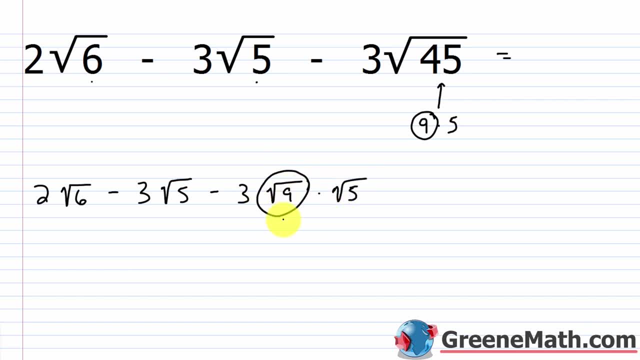 times the square root of 5.. The square root of 9 is 3.. So you basically have 3 times 3,, which is 9.. So let's rewrite this as 2 times the square root of 6, minus 3 times the square root of 5,. 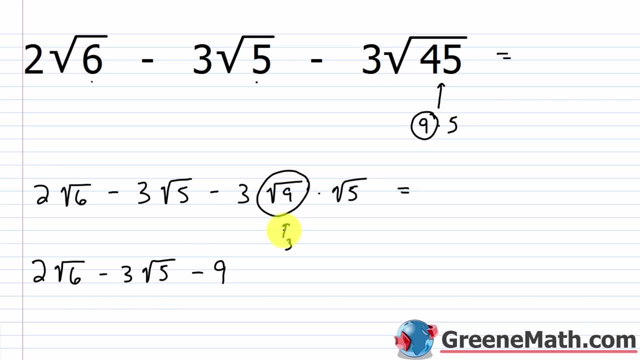 then, minus we said 3 times 3, would give us 9, times the square root of 5.. Although I don't have like radicals everywhere, I can combine these. These are like radicals. So what we can say is: we'd have 2 times the square root of 6,. 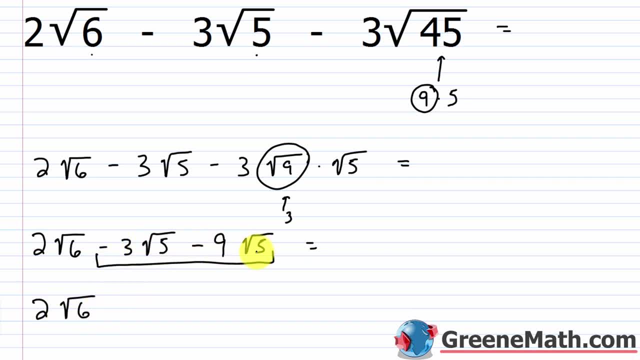 negative 3 times the square root of 5, minus 9 times the square root of 5.. You just take negative 3 and subtract away 9, that would give us negative 12, and then it's times that common radical, which is the square root of 5.. 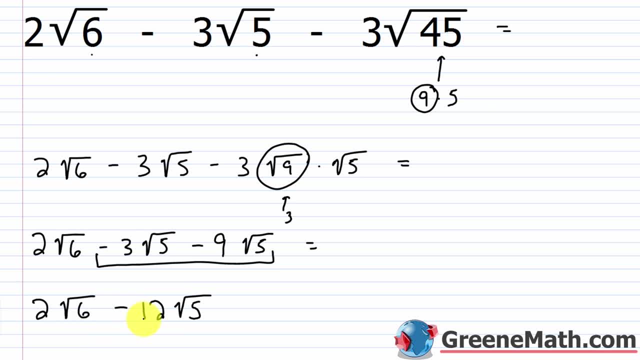 So we end up with 2 times the square root of 5, minus 3 times the square root of 6, minus 12 times the square root of 5.. Alright, let's take a look at another one. So we have 2 times the square root of 20, minus the square root of. 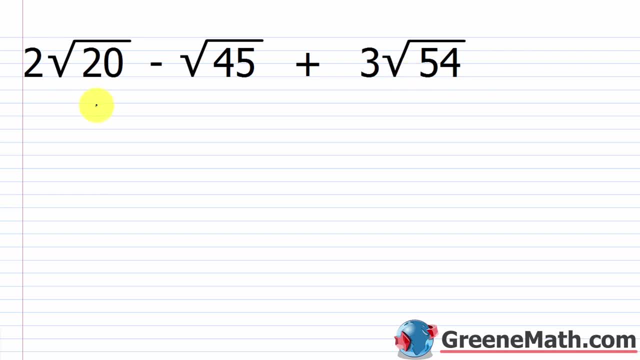 45, plus 3 times the square root of 54.. So I can simplify this: This is what 5 times 4.. We can simplify this: This is 5 times 9.. And we can simplify this: This is: 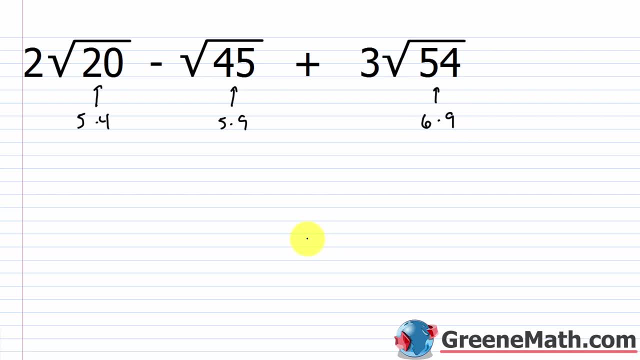 6 times 9.. And so there's a perfect square as a factor of each of these. So let's go ahead and simplify. So we would have 2 times the square root of 5, times the square root of 4,. 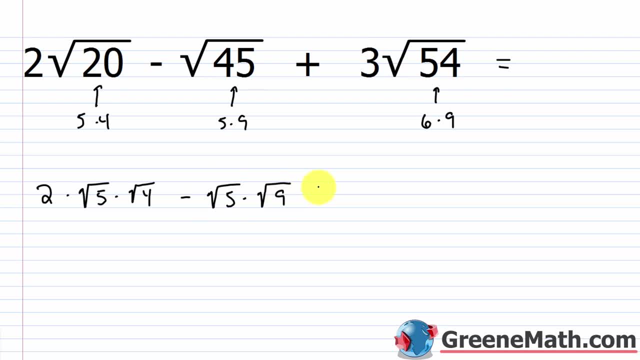 minus the square root of 5, times the square root of 9, plus 3 times the square root of 6, times the square root of 9.. So we know that this is 2.. This is 2.. We know that this is 3.. 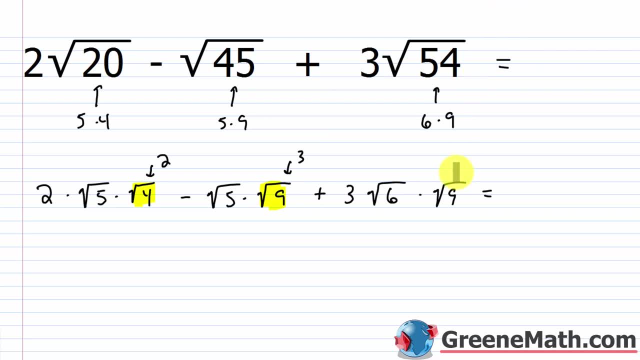 This is 3.. And we know again that this right here is 3.. So what do we get? You'd have 2 times 2,, which is 4.. Times the square root of 5, minus, you'd have 3 times the square root of 5, plus, you'd have 3 times 3,, which is 9, times the square root of 6.. 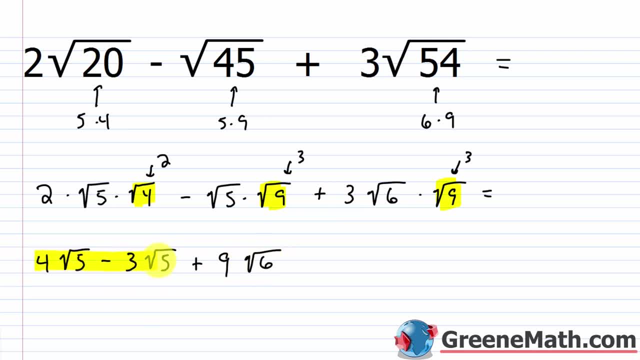 So, although we can't combine everything, we can perform this operation here. So we're going to do 4 minus 3, which would give us 1.. Now, if 1 is in front, I don't need to write it. I could put 1 times the square root of 5,. 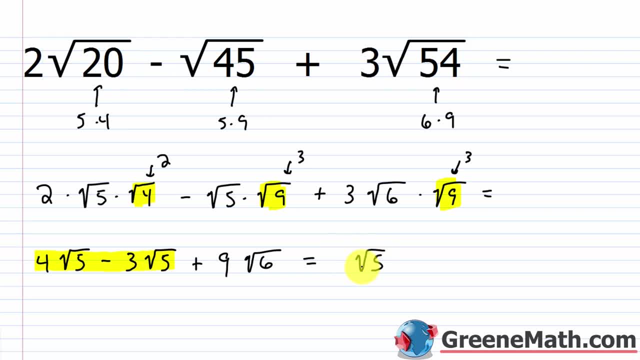 or I could just put square root of 5.. 1 times anything is just itself. Then, plus, we're going to have 9 times the square root of 6.. Now I can't simplify this any further. These are not like radicals, so this is just my answer. 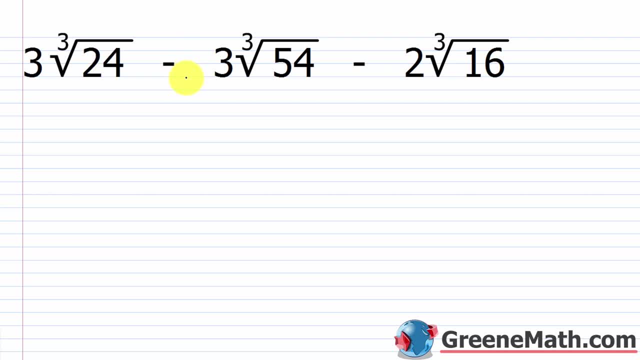 Alright. so let's take a look now at 3 times the cube root of 24, minus 3 times the cube root of 54, minus 2 times the cube root of 16.. So now we're working with cube roots. 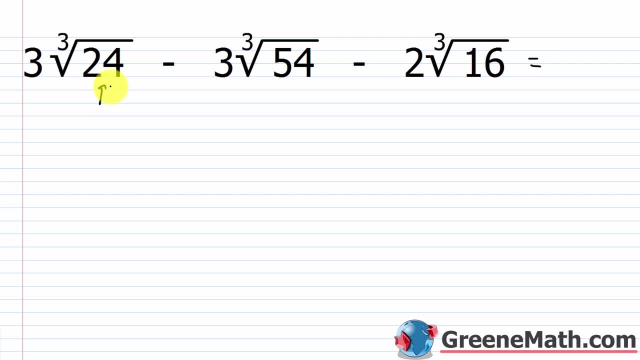 So you think about 24, and you're looking for a factor that would be a perfect cube: A number that, when multiplied by itself 3 times, gives you that number back. So when I think about 24,, are there any factors that would be a perfect cube? 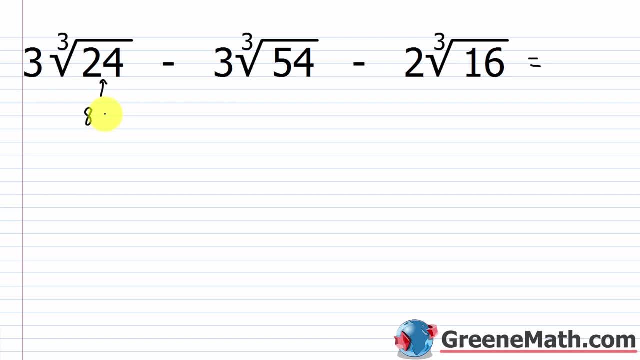 Well, yeah, 8 would be. 8 is too cute. So 8 times 3, 54,- let's think about that. 54 has 27.. So 54 is 27 times 2.. And 27 is what It's. 3 cubed 3 times 3 is 9,. 9 times 3 is 27.. 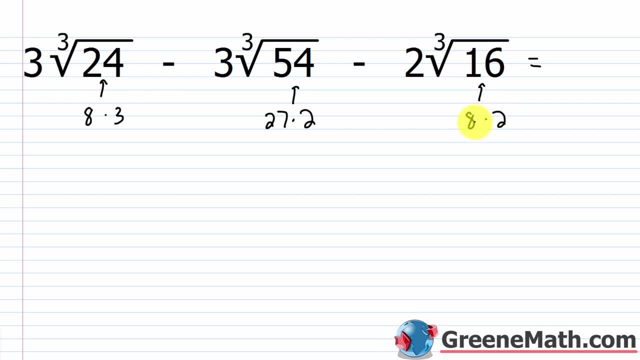 And 16 is what It's: 8 times 2.. 8 is a perfect cube and again it's too cute. So let's go ahead and simplify. We'll have 3 times the cube root of 8, times the cube root of 3,. 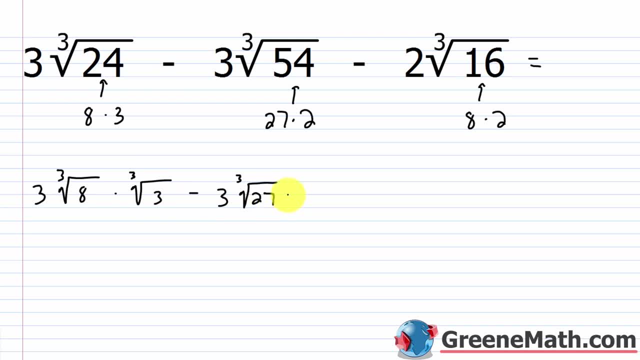 minus 3 times the cube root of 27 times the cube root of 2, minus 2 times the cube root of 8 times the cube root of 2.. So we look at what we can do here. We know that this would simplify. 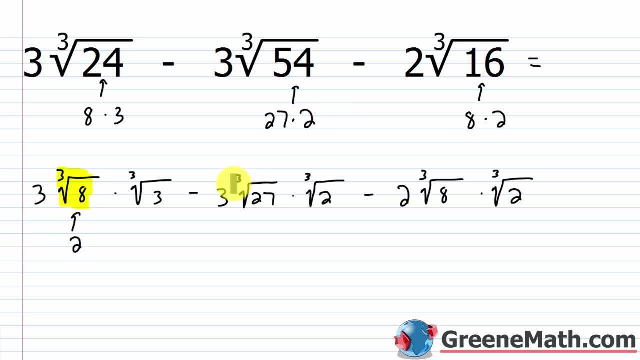 It would be 2.. We know that this would simplify right here. it would be 3 and again we know that this would simplify, it would be 2. so let's go through and crank this out: 3 times 2 would be 6, so you would. 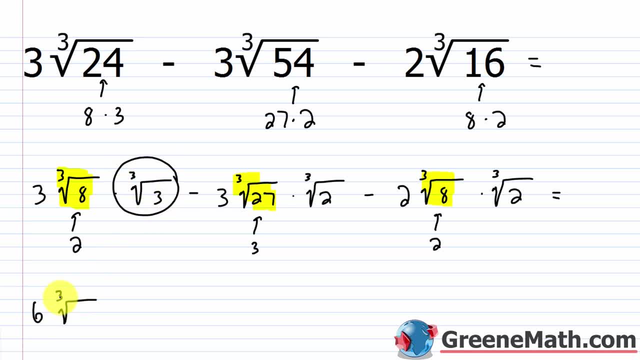 have 6 times this cube root of 3. then minus, 3 times 3 is 9 times this cube root of 2. then minus, you'd have 2 times 2, which is 4 times the cube root of 2. now, we don't have like radicals everywhere, but what we can do is we can combine. 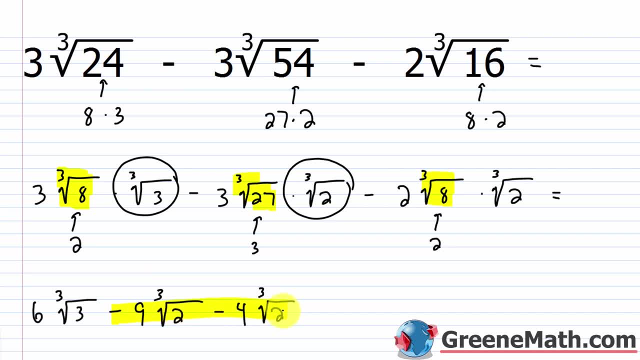 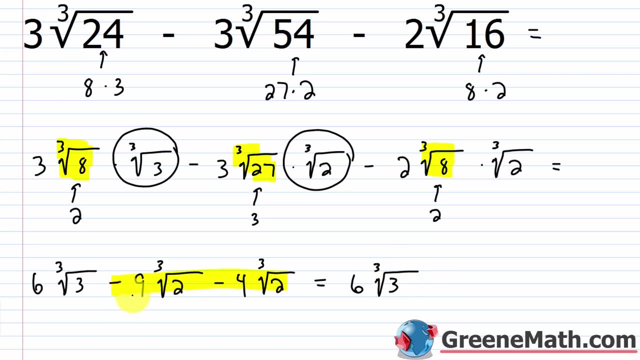 these two because you have cube root of 2 and cube root of 2, so you start out by just writing 6 times the cube root of 3, then you have negative 9 minus 4, which is negative 13, or minus 13 times that common radical which is the cube root of 2. all right, for the next. 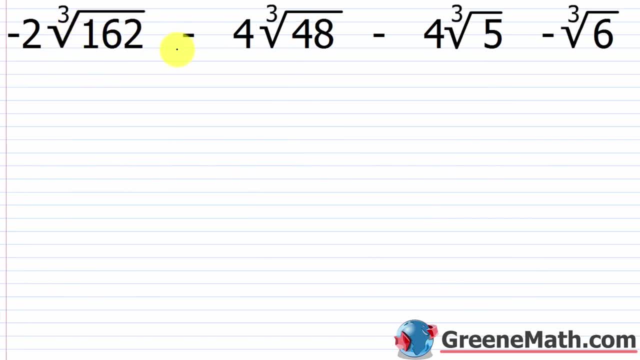 one. we have negative: 2 times the cube root of 162 minus 4 times the cube root of 48, minus 4 times the cube root of 5 minus the cube root of 6. so let's take a look at 162. we would first want to factor that. so what would this factor? 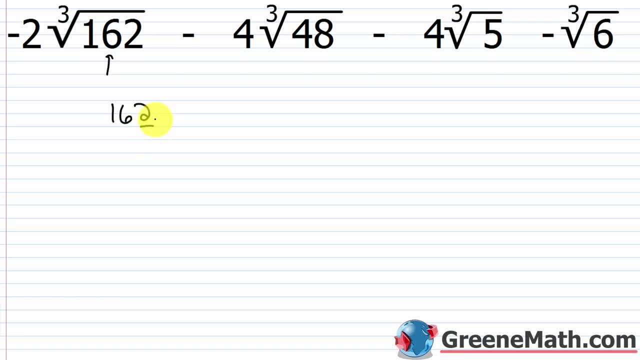 into. well, it's divisible by 2, so let's just start with that. if I divided this by 2, I would get 81. so 2 is prime. 81 is what it's 9 times 9. we know, 9 is what it's 3. 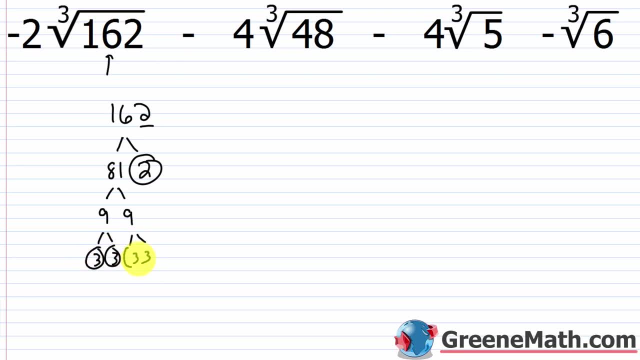 times 3, so we do have a perfect cube here. we have 3 times 3 times 3, which is 27 times what's left, which is 3 times 2 or 6. so let's factor this as 27 times 6, so we'll say that this equals negative 2. 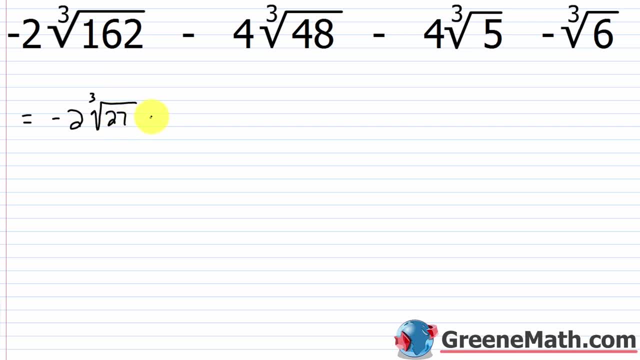 times the cube root of 27, times the cube root of 6, then minus, you have your 4 out in front now for 48, we could factor that as 8 times 6. we already know that 8 is a perfect cube. so let's do the cube root of 8 times the cube root of 6, then minus. 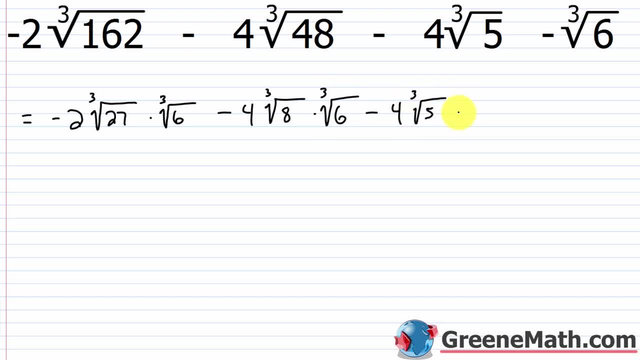 you have 4 times the cube root of 5, then minus the cube root of 6. so we know that we can simplify this guy right here: this is 3. we know we can simplify this guy right here, this is 2. so what would we get if? 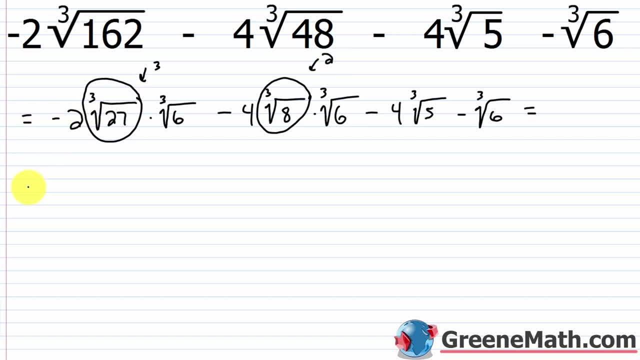 we do that, negative two times three would be negative 6. then times the cube root of 6, then you have minus. we know this is 2, so you'd have 2 times 4, that 8 then times the cube root of 6, then minus 4 times the cube root of 6. 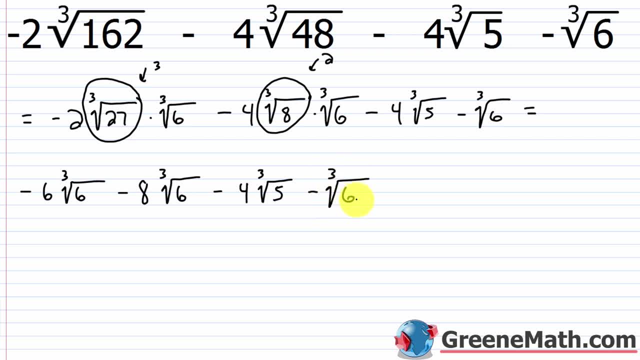 of 5, then minus the cube root of 6.. Now, what can we combine When we think about, like radicals? we have the cube root of 6, the cube root of 6, and the cube root of 6.. 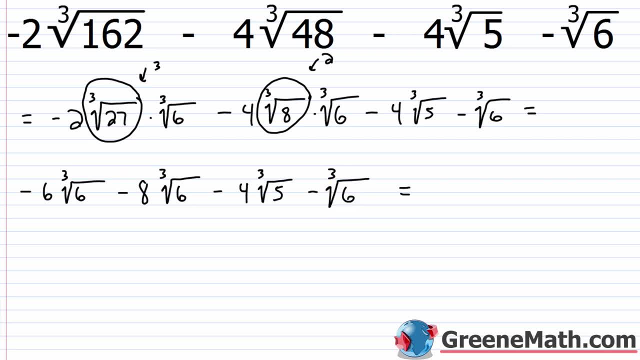 So I'm just looking at what's multiplying in front. So negative 6,, negative 8, and then this is understood to be negative 1.. So it's just like if I had a negative x, this is understood to be a negative 1 times x. 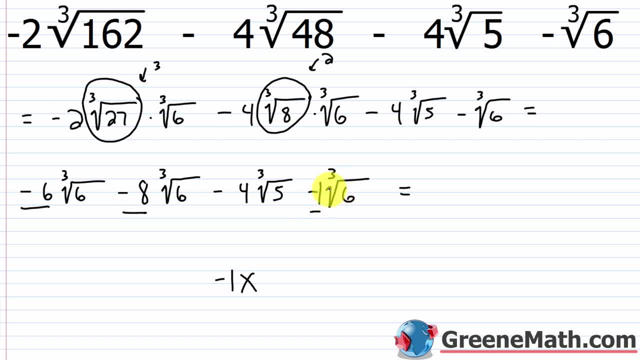 Same thing here. if I have a negative out in front, it's like having a negative 1 multiplying that. So I would have negative 6 minus 8, that's negative 14, then minus another 1, that's negative 15,. 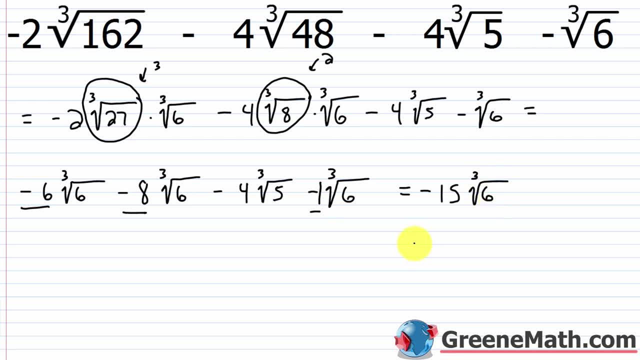 times this cube root of 6. Then we would have minus 4 times the cube root of 5.. And then these are not like radicals, so we can't simplify this any further. All right, so now we have negative 2 times the cube root. 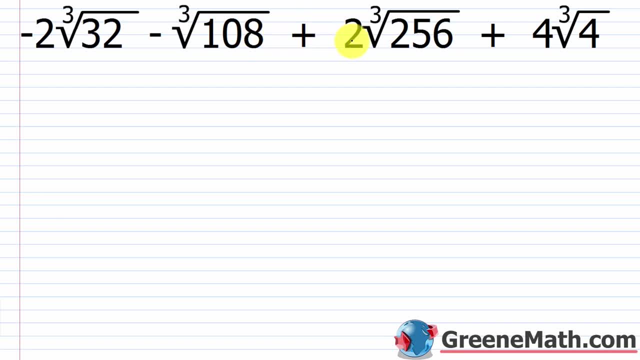 of 32.. Minus the cube root of 108, plus 2 times the cube root of 256, plus 4 times the cube root of 4.. All right, so we think about 32.. We know that there's a perfect cube there. 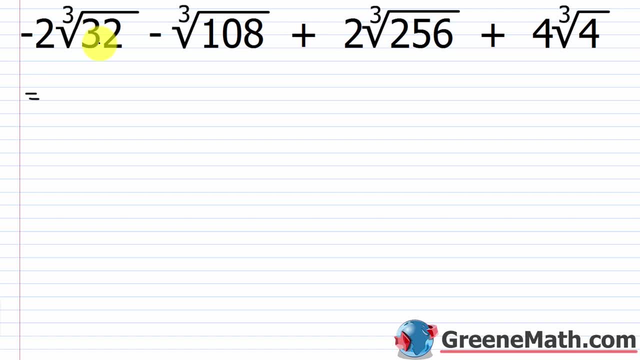 32 is 8 times 4.. All right, again, 8 is a perfect cube. So we put negative 2 times the cube root of 8, times the cube root of 4.. Then minus For the cube root of 108, we don't think about 108. 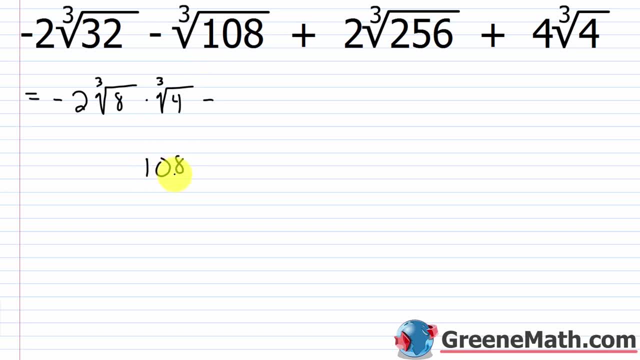 that often. So let's factor that guy. So 1 plus 0 plus 8 is 9.. So we know this number is divisible by 9.. It's also divisible by 3.. So if we went ahead and divided it by 9,, 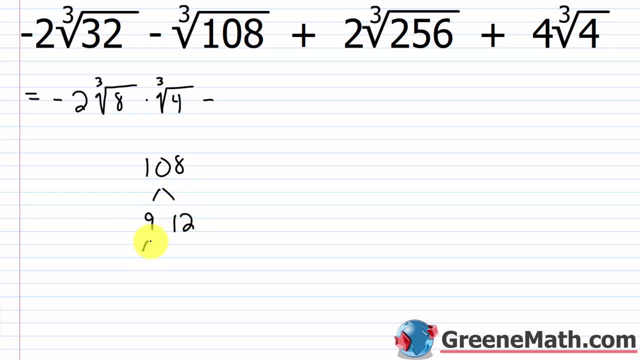 we could do 9 times 12. Then we could see that 9 is 3 times 3, and 12 is what It's 4 times 3.. And you could stop there, because you know you basically have 27 times 4.. 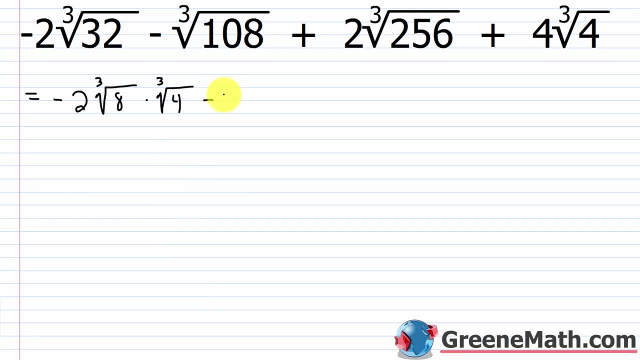 27 is a perfect cube. so we could say we have minus the cube root. So we have minus the cube root of 27 times the cube root of 4. Then plus We'll have 2 times the cube root of for 256,. 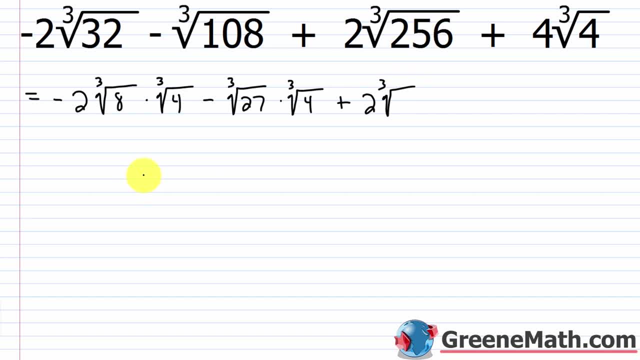 we don't really need to factor it At this point. you should know it's 2 to the eighth power. So if you're thinking about a perfect cube, you want an exponent that would be divisible by 3.. OK, So 8 wouldn't be. so you start going down. 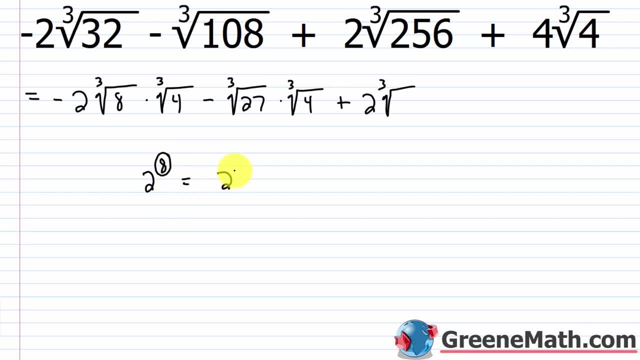 7 wouldn't be, 6 would be. So you're going to have to break this up into 2 to the sixth power times 2. squared Right, 2 to the sixth power is 64. So you can put the cube root of 64 times the cube root of 2. 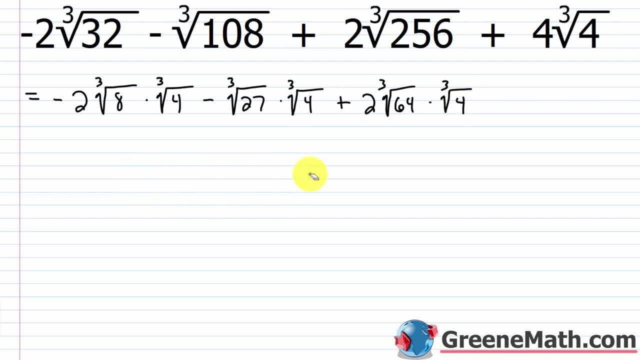 squared, which is 4.. Let's erase this, Then plus, You'd have 4 times the cube root of 4.. Nothing I could really do with that, All right. So now we look at what we can simplify. So this guy right here: 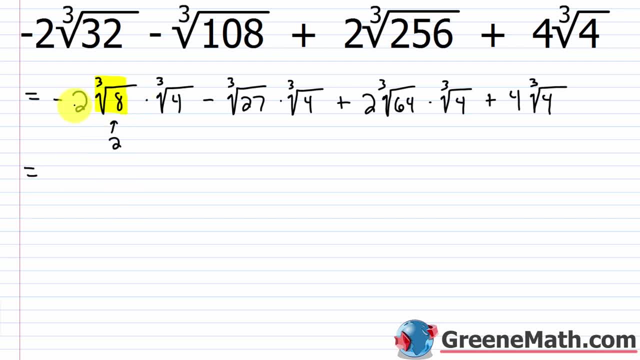 Here is going to be 2.. So negative 2 times 2 is negative 4.. And then times what's left, which is the cube root of 4. Then we can simplify this guy right here. That's going to be 3.. 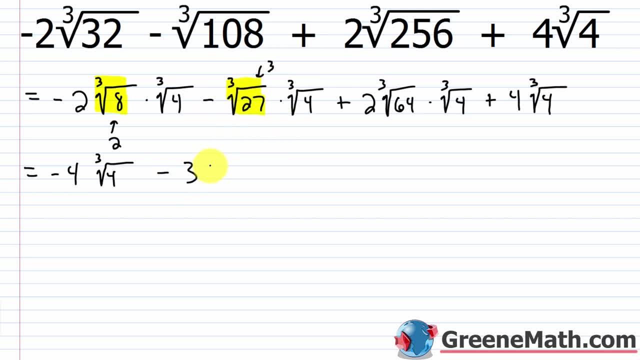 So you'd have negative 3.. So minus 3 times the cube root of 4.. Then, plus This guy right here, the cube root of 64 is 4.. So you'd have 2 times 4, which is 8, times the cube root of 4.. 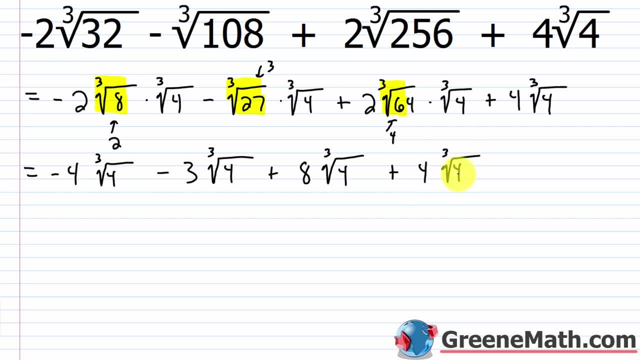 Then, lastly, you have plus 4 times the cube root of 4.. So now we have like radicals everywhere. So I'm just going to go through and see what we can combine. We have negative 4 here and positive 4 here. 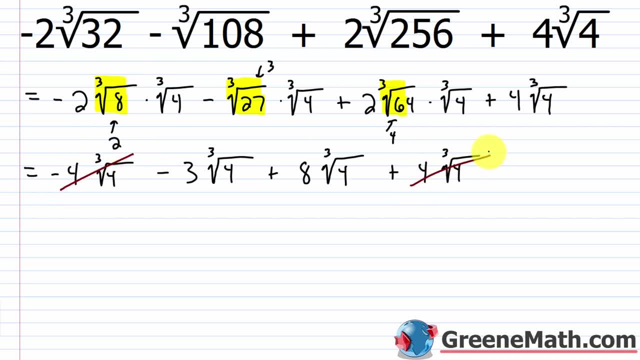 So essentially, this would cancel. with this, Those would become 0.. All I'm really left with is negative 3 plus 8, which is 5, times this common radical which is the cube root of 4.. Hello and welcome to Algebra 2, Lesson 58. 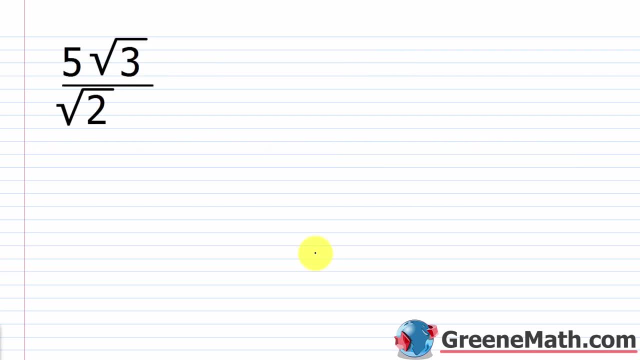 In this video we're going to learn about rationalizing the denominator. So for the majority of you, you took Algebra 1 before jumping into this Algebra 2 course And I know most of you have seen rationalizing the denominator before. But again, when you get into Algebra 2 or even college, 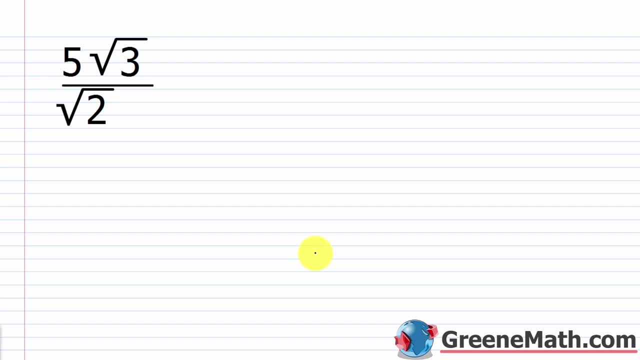 algebra. there's just a lot of topics that you go over again, So it's not something that you should be bored with. Take the time, Take the time to again cover this again and make sure you have a complete understanding of it. 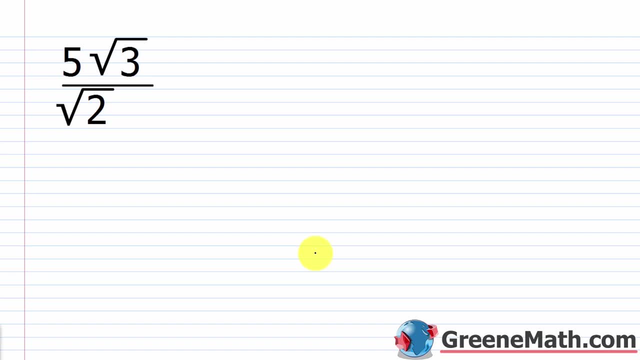 And if it's something you're seeing for the first time, this is not something that's super difficult. Some of the examples will get a little bit challenging, though, All right, So let's start off with something kind of simple. So we have 5 times the square root of 3 over the square root of 2.. 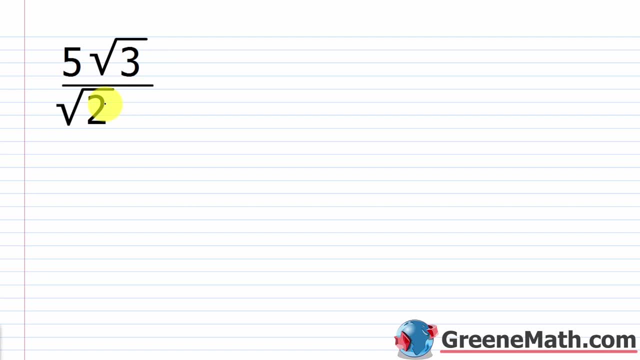 So the first question we would ask is: is this simplified? So I would relate this to when we work with fractions. If we had something like 3 times the square root of 3 over the square root of 2, then we would have the same thing. 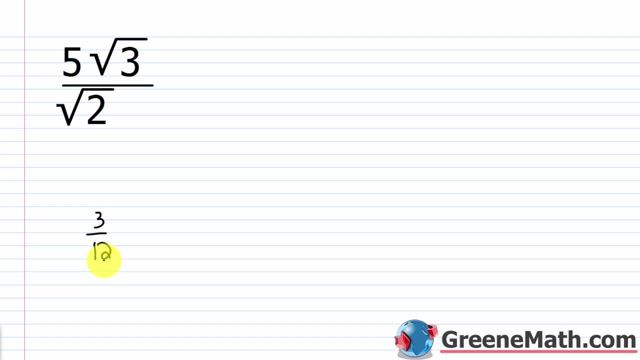 If we had something like 3 times the square root of 3 over 12, we didn't report that. We wanted to simplify this and say, OK, well, 3 divided by 3 is 1,, 12 divided by 3 is 4.. 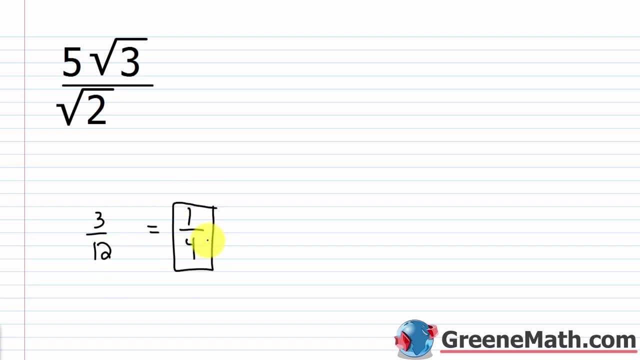 So the simplified answer here would be 1. fourth, This is simplified, But mathematically these two have the same value. They're both equal to 0.25 in decimal form. It's going to be kind of a similar experience over here. 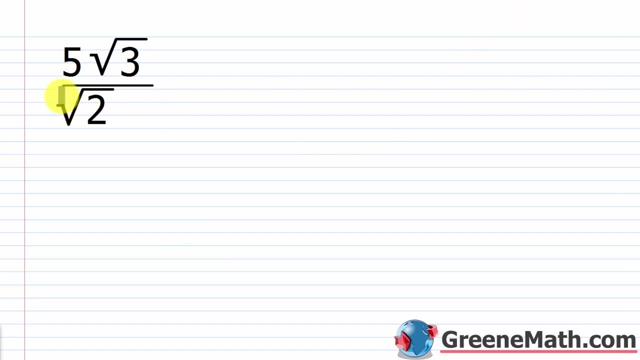 Our rule is: we don't want a radical in the denominator. So here we have the square root of 2, which is a radical. So, in order to simplify this, what we do is a little trick: We're going to multiply the numerator and denominator by the square root of 2.. 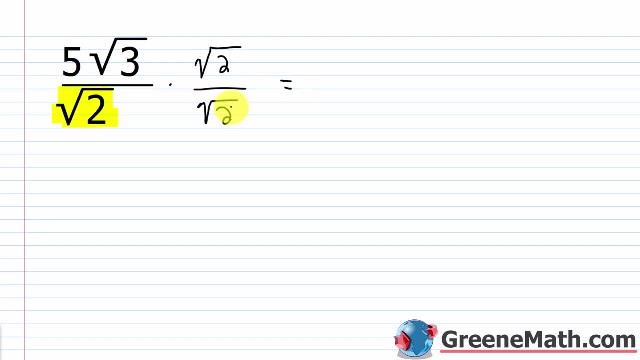 Now what's that going to do for us? The square root of 2 times the square root of 2 is the square root of 4.. And the square root of 4 is 2.. So what we did is we took an irrational number like the square root of 2.. 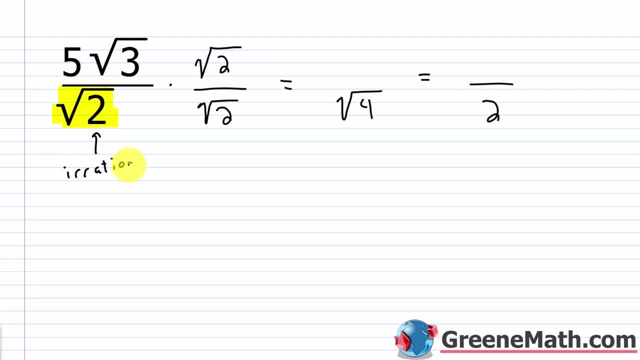 Let me write that this is irrational And we made it into a rational number, which is 2.. Henceforth the term rationalizing the denominator. We go from an irrational number, that's a denominator, to a rational number, that's our denominator. Now I can't just do something to the denominator without doing the same thing to the numerator. 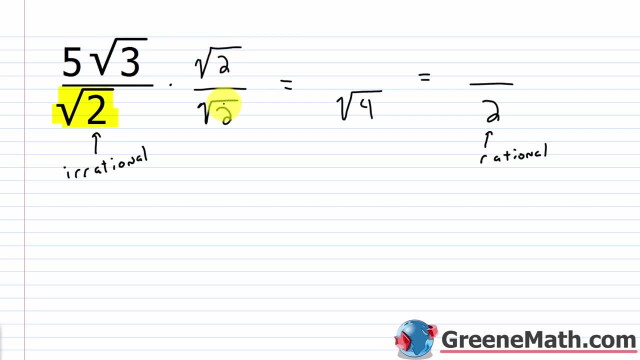 Remember, just like we work with fractions, Same nonzero number over 2.. Same nonzero number over itself is 1.. So this has a value of 1.. And if we multiply by 1, something is unchanged. So you'd essentially have 5 times square root of 3 times square root of 2.. 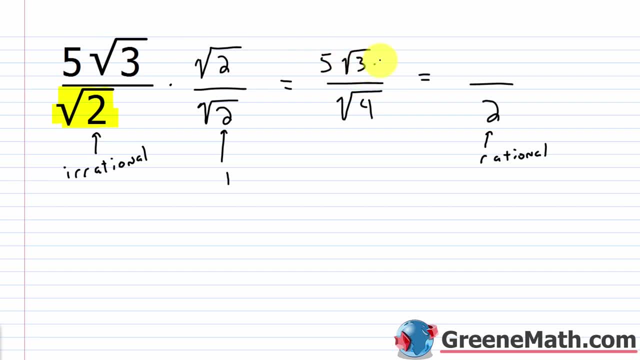 So we'd have 5 times square root of 3, times square root of 2, which simplifies to 5 times the square root of 6.. So some of you will say, well, how come there's a radical in the numerator? 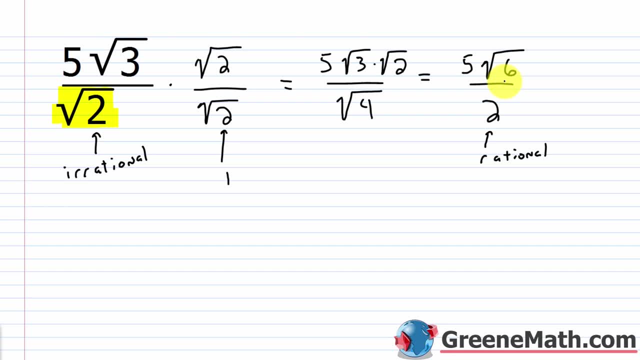 Why is that allowed? The reason for this is When this rule was invented On how to simplify A radical, They didn't work with calculators. Now I can take this guy right here And this guy right here And I can punch it up on a calculator in an equal amount of time. 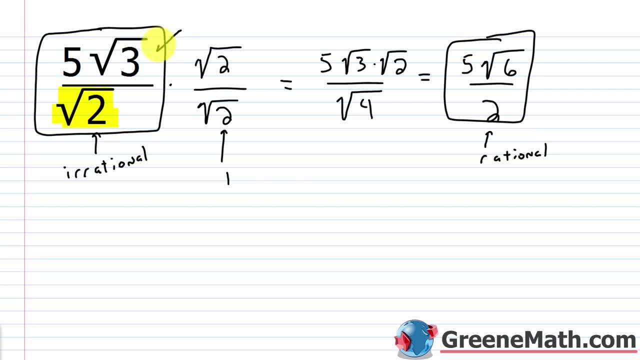 If I didn't have a calculator- This one right here on the left- This guy would take longer to calculate Than this guy. Now, the rule has still stuck around, And you're expected to know how to do this in almost every math class. 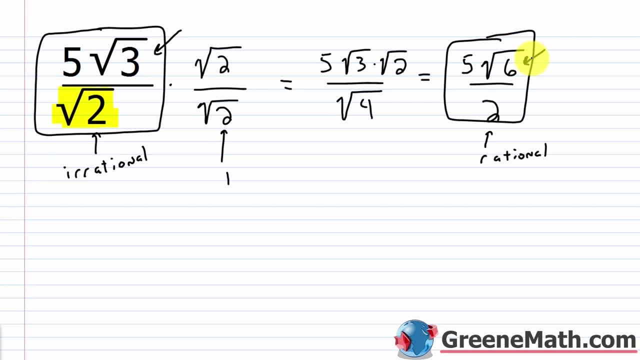 So it's something you just need to learn how to do, But mathematically, This guy right here And this guy right here, They have the same value. It's just like when we looked at 3 twelfths And 1 fourth. 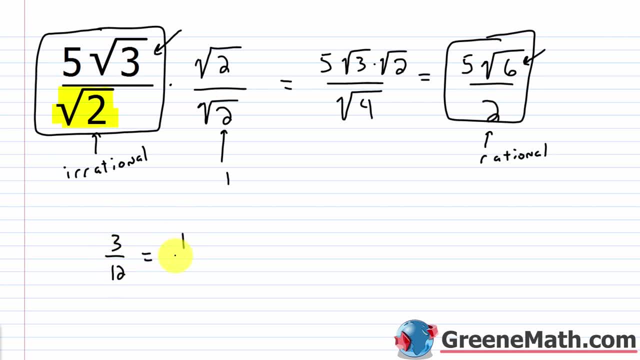 Right, They are the same mathematically. One is simplified, One is not. All right, Let's take a look at another. So suppose you see something like this: 4 times square root of 9.. Over 2 times square root of 6.. 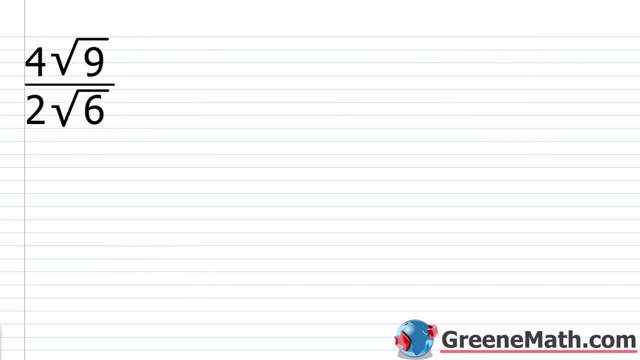 Well, the first thing is: You know you can cancel this 4.. With this, 2. Right, 2 divided by 2 is 1.. 4 divided by 2 is 2.. So you know you can cancel this 4.. 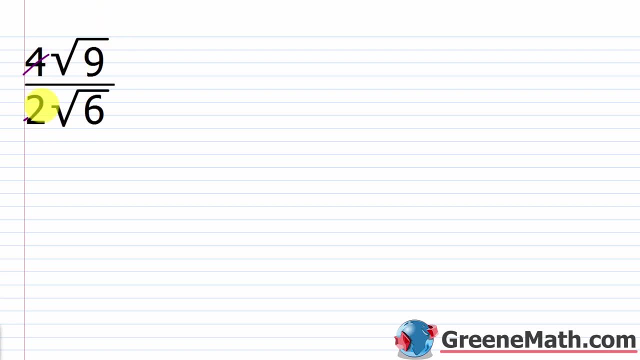 With this: 2.. Right: 2 divided by 2 is 1.. 4 divided by 2 is 2.. So you know you can cancel this 4.. With this: 2.. 4 divided by 2 is 1.. 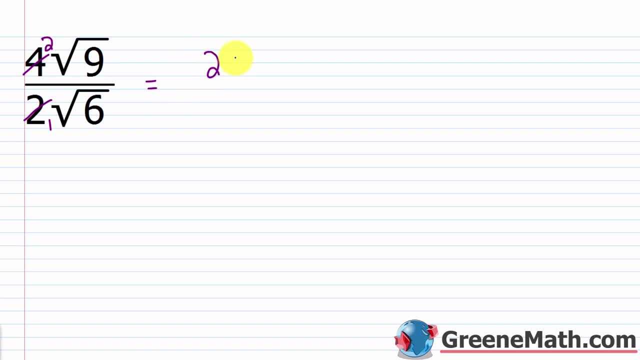 4 divided by 2 is 2.. So this would turn the problem into 2 times the square root of 9.. Over the square root of 6.. Now the next thing is the square root of 9 is 3.. So we can go ahead and simplify that and say we have 2 times 3, which is 6.. 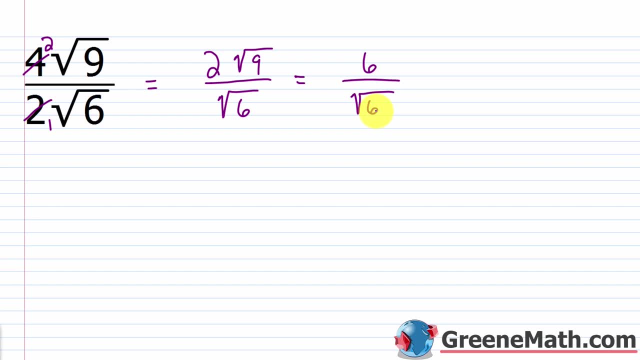 Over the square root of 6.. Okay Now, in order to report a simplified answer, We don't want a radical in the denominator, So, again, we're going to use our little trick: We're going to multiply this by the square root of 6.. 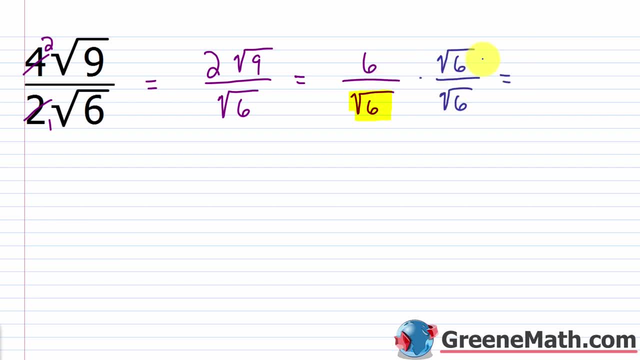 Over the square root of 6.. And what's going to happen is you'll have 6 times the square root of 6.. Over the square root of 6 times the square root of 6 is what It's: 6. Right. 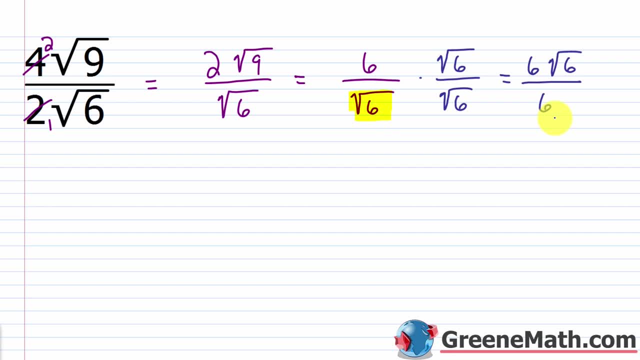 It would be the square root of 36.. The square root of 36 is 6.. Now, between the numerator and denominator, I can cancel a common factor of 6.. This is multiplication here. So I'm canceling common factors And what we're left with is simply the square root of 6.. 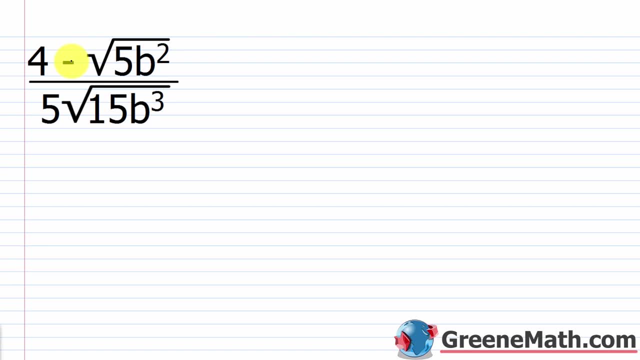 Alright, Let's look at another one. So we have 4 minus the square root of 5b squared Over 5 times the square root of 15b cubed. So a lot of things to simplify. first. You always want to think about what can I simplify? 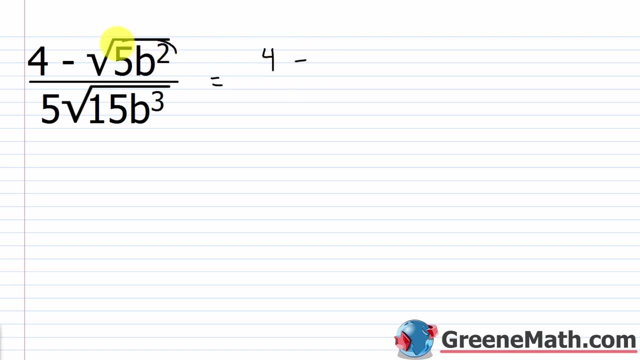 So we have 4 minus. Now this right here. you think about b squared. The square root of b squared is nothing more than b. Again, A quick way to do that is with exponents. If I have b squared And I'm taking the square root of that, 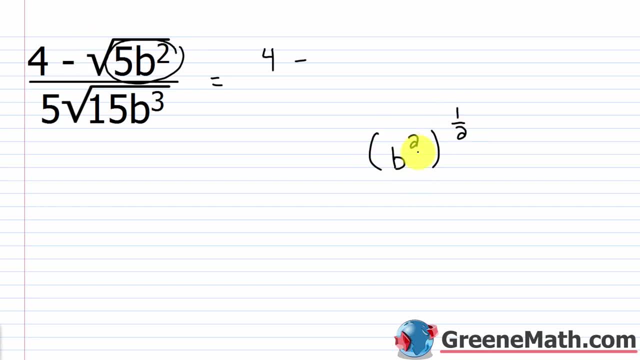 So this is like raising something to the 1 half power. You do power to power rule here. You have b raised to the power of 2 over 2.. Which is just b to the first power, or b. What's going to happen is. 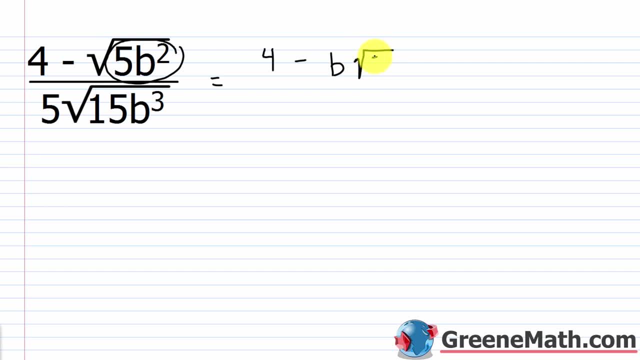 I'm going to pull a b outside And it'll be times the square root of 5.. And this is over Down. here I have 5. Which is multiplied by, You've got 15b cubed. Now, 15 is 5 times 3.. 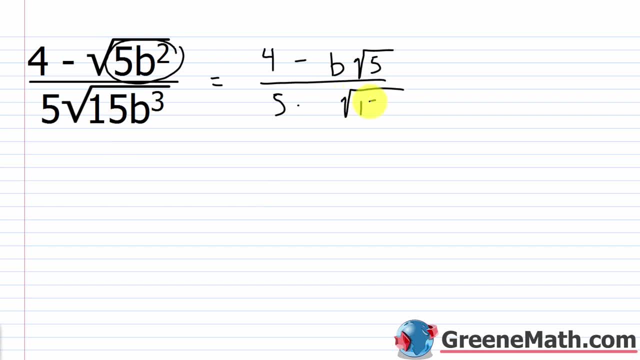 So I can't really do anything with that. So Let's stay underneath. But with b cubed again. If this guy right here is equal to or greater than the index, You know you can simplify that Right. I can separate that up into b squared. 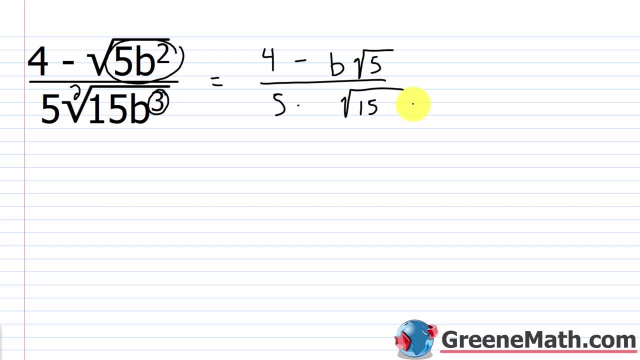 Multiplied by b. So if I wanted to go kind of a long way about this, I could say: this is the square root of b. squared times the square root of b- This guy right here- is b, So that could come out And I could erase this. 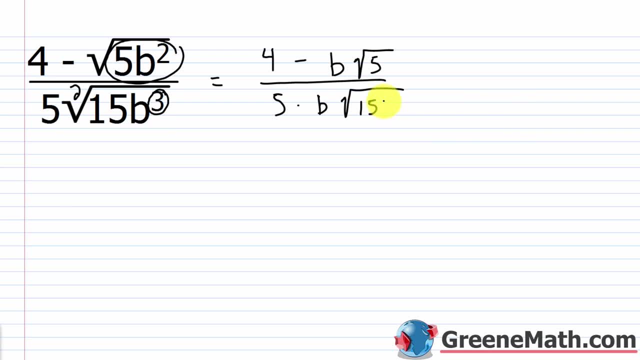 And if I'm multiplying by the square root of b, I could just write this underneath. So we've simplified that part as much as we can. But again, in the denominator There is a radical, So I'm not going to multiply by the entire denominator. 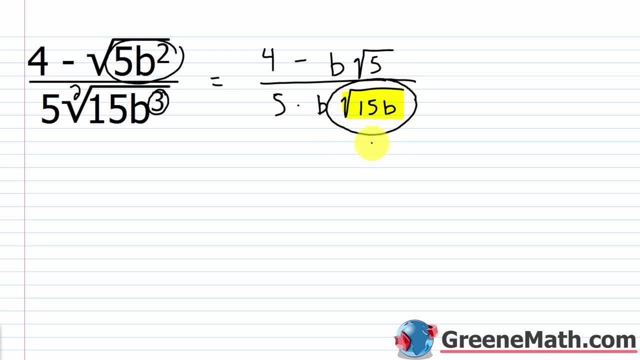 I'm just going to multiply by what I need to To get rid of that radical. So let's start that down here. We have 4 minus b times the square root of 5.. Over 5b times the square root of 15b. 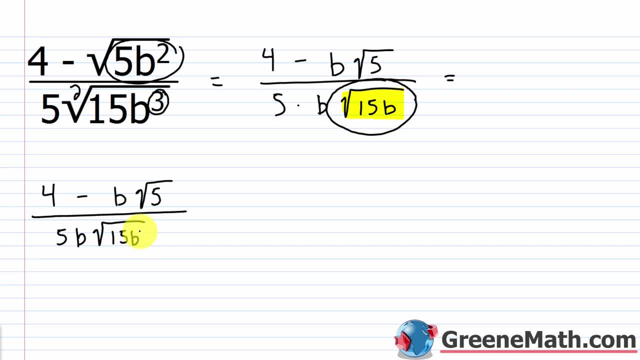 Okay, Now what I'm going to do. I'm going to multiply the numerator and denominator By this guy right here, So the square root of 15b Over the square root of 15b. Now there's a minus sign here. 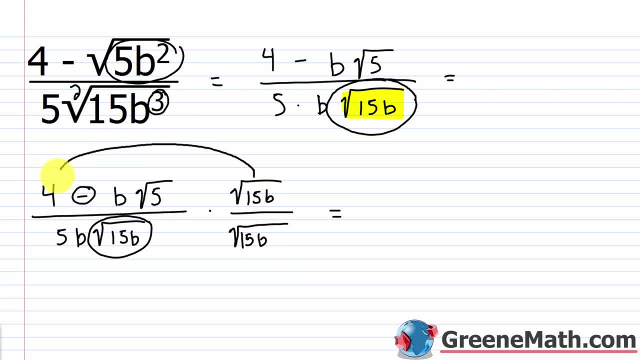 If I'm going to do this properly, I'm going to use my distributive property. This is going to be multiplied by this And that's going to be multiplied by this. So you'd have the square root of 15b Multiplied by 4.. 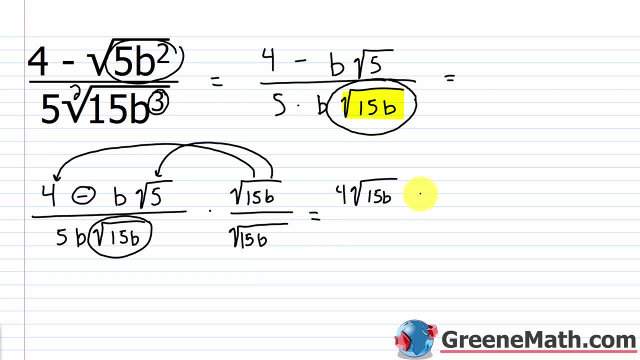 So 4 can just go out in front. Then minus I've got b times the square root of 5 times the square root of 15b. So b is out in front. Times the square root of 5 times the square root of 15b. 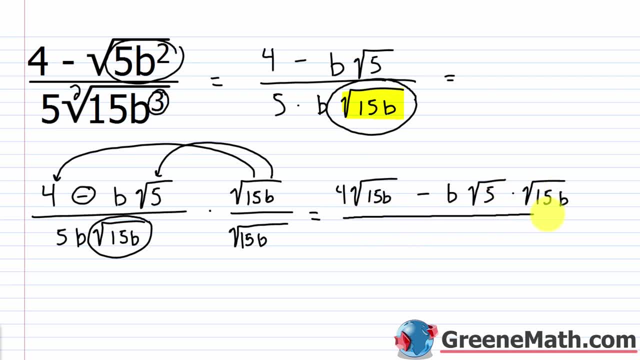 And this can be simplified further, but we'll do that in a minute. This is over. Now, down here, I've got this: 5b Multiplied by You have the square root of 15b times the square root of 15b. 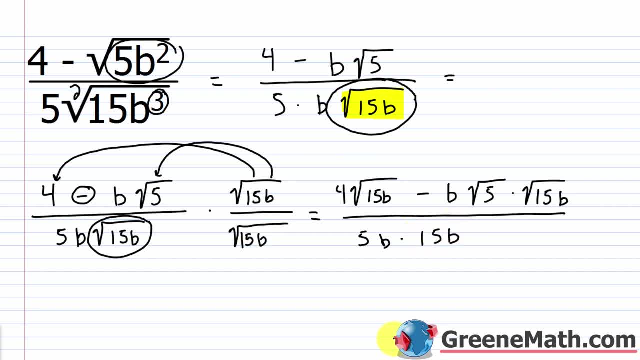 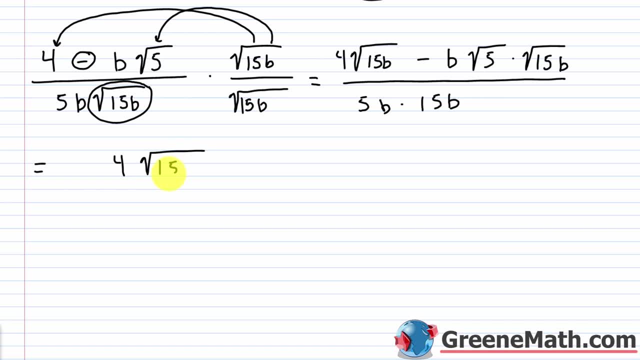 Which is just 15b. Okay, So let's further simplify Now. So in the numerator we have 4 times the square root of 15b. Nothing I can really do with that. 15 is 5 times 3.. 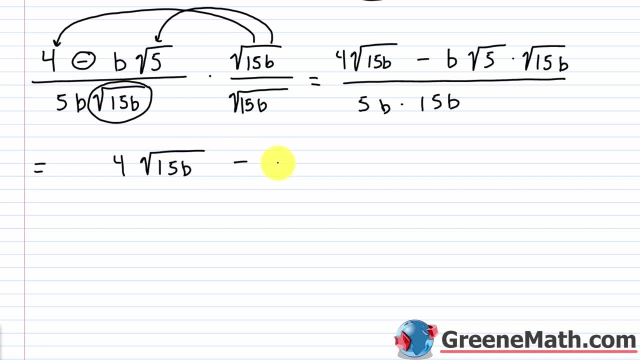 B is just b, Can't really do anything. Then minus. Then for this guy right here, I have b times the square root of 5.. Then I'm going to break this up into the square root of 5 times the square root of 3 times. 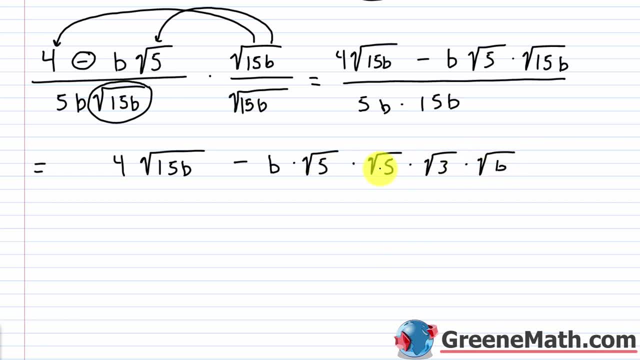 the square root of b, Now square root of 5 times square root of 5, is 5.. So I might as well just erase this and put 5.. And then there's really nothing else I can do with the rest of that. 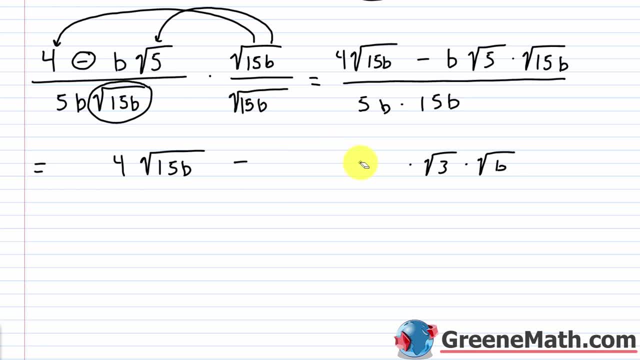 So if I want to clean this up, I could put minus 5b, Minus 5b Times, the square root of 3b, Times the square root of 3b. Then this is over. You've got 5b times 15b. 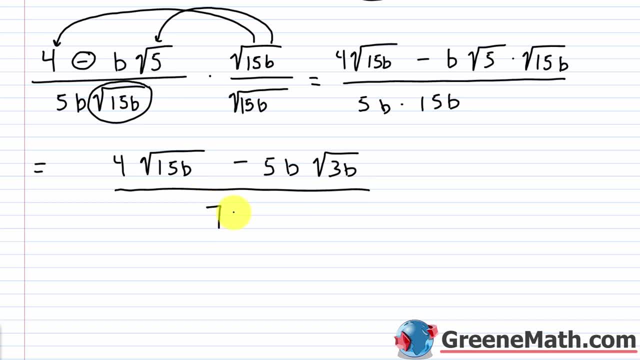 Really all I can do is say that's 75b squared. The last thing I want to do Is see if there was anything that would cancel between numerator and denominator. Remember, you've got subtraction here. This is not multiplication, So I would have to factor something from both terms in the numerator. 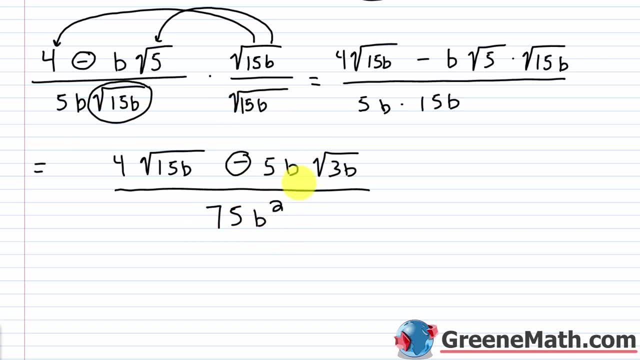 I'd have to factor something out to see if it would cancel here. So when I look at this, there's not really anything I could do that would make an impact. Some of you will say: well, in the numerator you could factor out the square root of 3b. 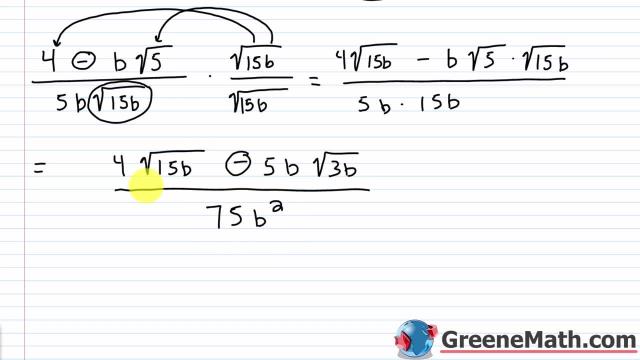 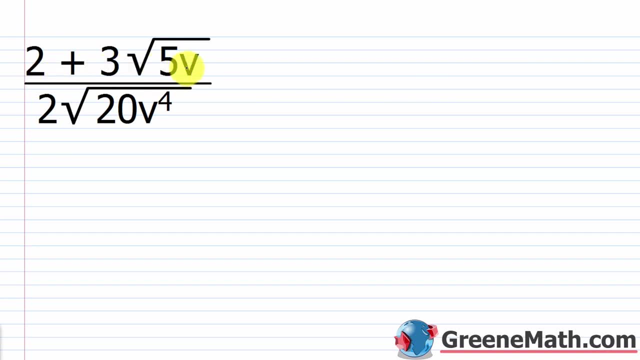 You could, but there's nothing to cancel that with down here, So this would be as simple As we can make this. Alright, let's take a look at another one. So we have 2 plus 3 times the square root of 5b. 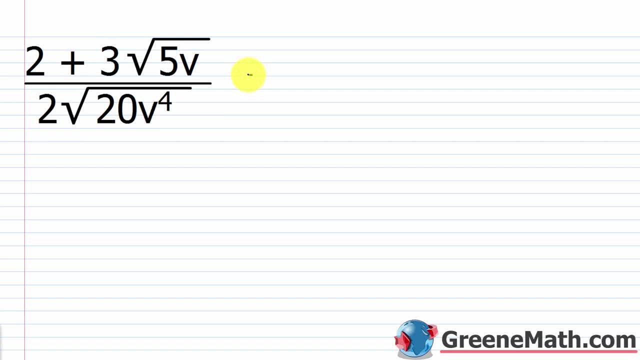 Over 2 times the square root of 20b to the fourth power. So in the numerator, nothing really to simplify, So just 2 plus 3 times the square root of 5b. Now in the denominator we have 2 times for the square root of 20b to the fourth power. 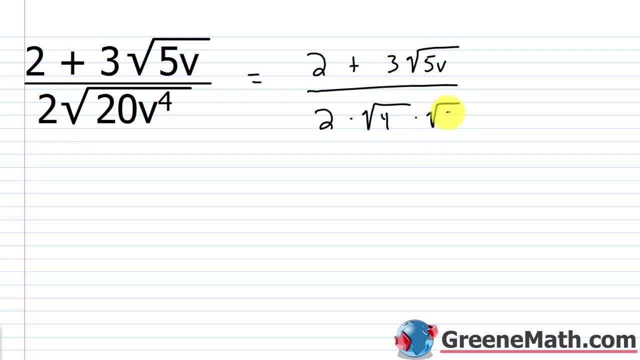 We'll break that up into the square root of 4. Times, the square root of 5. Times, the square root of v to the fourth power. So we can do some simplifying now: 2 plus 3 times the square root of 5b. 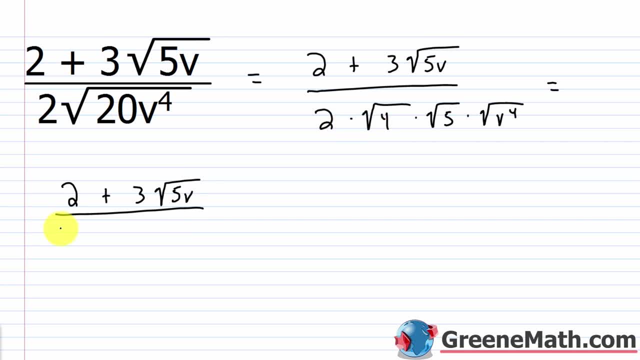 Over. the square root of 4 is 2.. So 2 times 2 would be 4.. So let's put a 4 out in front. Then the square root of v to the fourth power is v squared. Let's put a v squared next to that. 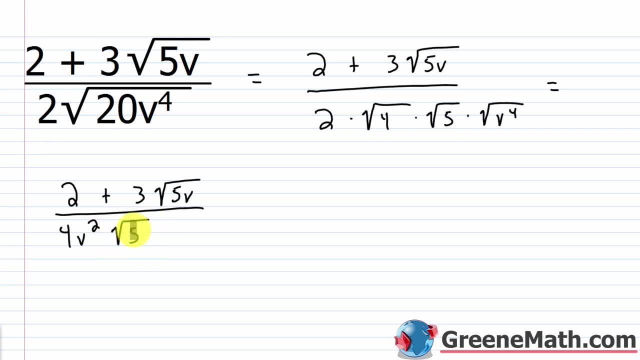 And then we're left with this square root of 5.. So this is pretty easy to clean up. I have a radical in the denominator that I want to kind of get rid of, So all I'm going to do is multiply the numerator and denominator by that square root of 5.. 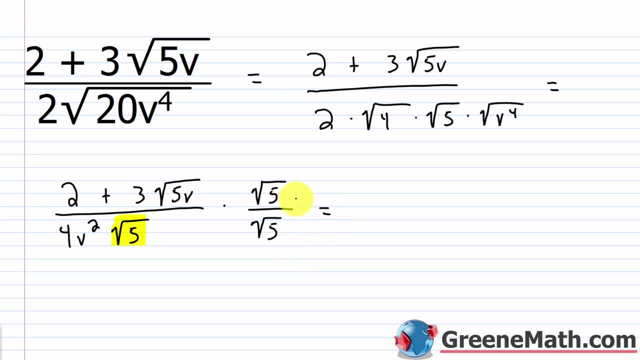 All right. So what's going to happen? Again, I've got to use my distributive property because I have this plus here. So square root of 5 times 2 is just 2 times square root of 5.. Then plus the square root of 5, multiplied by 3 times the square root of 5v, you really 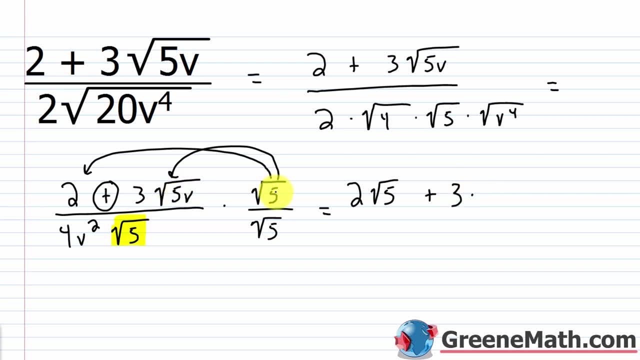 say So, let's put a plus here. So 5 times the square root of 5, times the square root of 5 is 5.. So 3 times 5 would be 15.. So let's just write 15.. 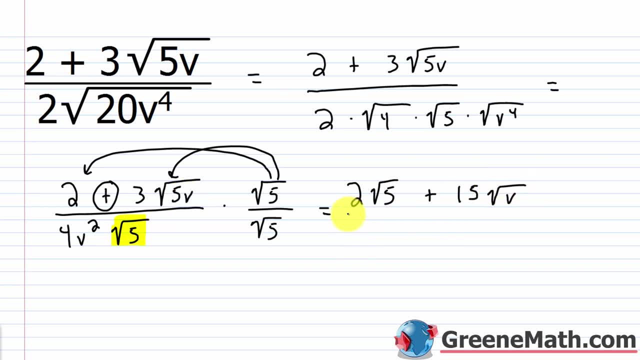 And then the thing that would be left would be the square root of v. okay, So times the square root of v, Then, over down here, square root of 5 times the square root of 5 is 5.. 5 times 4v squared would give us 20v squared. 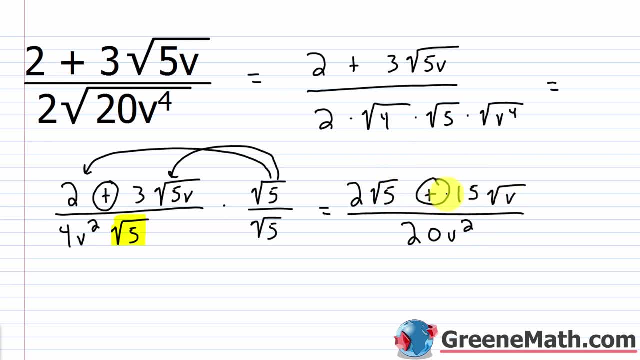 You're looking, if you want to cancel here, because there's this plus sign you'd have from both these terms here to be able to cancel it with something in the denominator. We don't really have anything. You have two and you have 15.. 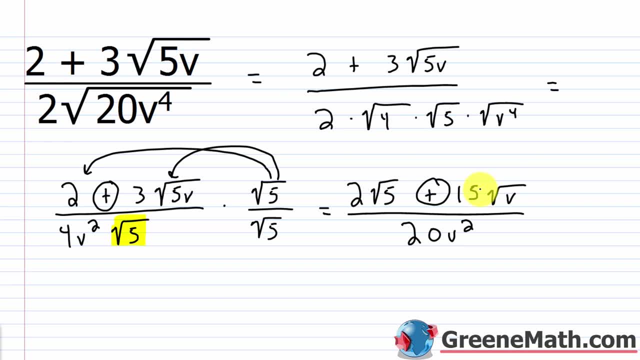 You have square root of five and you have square root of V, So nothing really I can pull out there that I could cancel with that 20 V squared. So this is simplified: Two times square root of five plus 15 times square root of V. 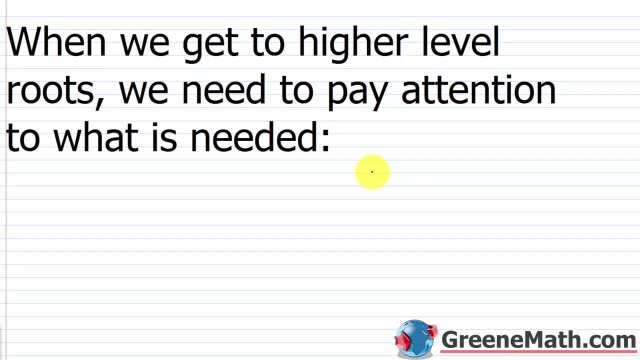 over 20 V squared. All right. so now let's talk about something that's a little bit more complex, which is dealing with this when we have higher level roots. So when we get to higher level roots, we need to pay attention to what is needed. 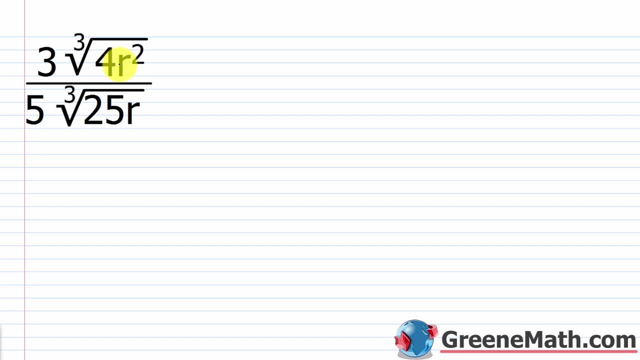 We think about something like this: We have three times the cube root of four R squared over five times the cube root of 25 R. This is one thing that you really gotta pay attention to. So you're looking at this and you're saying: 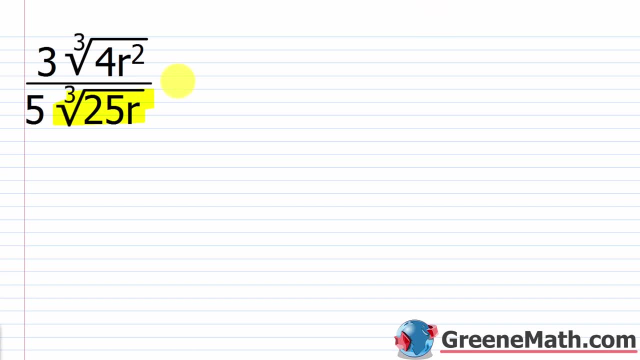 okay, I wanna simplify this. A lot of students will just start out and go: okay, you know what? I'm gonna multiply this by cube root of 25 R squared. I'm gonna multiply this by cube root of 25 R over cube root of 25 R. 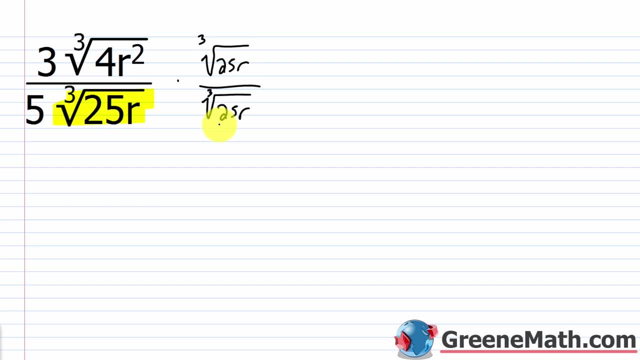 Now, 25 times 25 is 625.. That is not a perfect cube. It's a perfect fourth, but not a perfect cube. So again, when you see something like this, you want to factor things and kind of think about stuff. 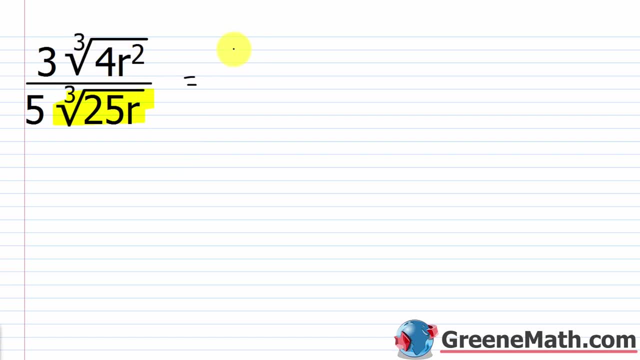 So in the numerator there's nothing really I can do to simplify. So three times the cube root of four: R squared. We know four is a perfect square but not a perfect cube. R squared is a perfect square but not a perfect cube. 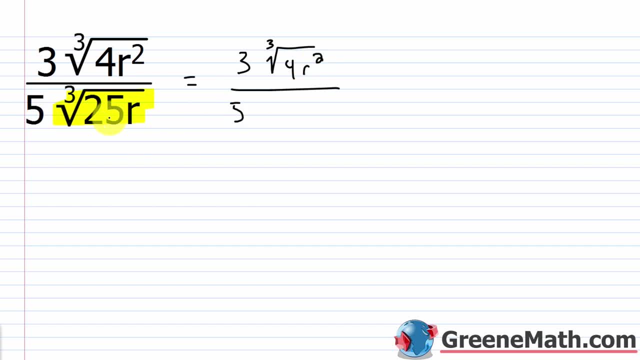 So we move on to the denominator. We have our five, and then we're gonna break this up. So times the cube root of five times the cube root of five, five times five is 25, and then times the cube root of R. 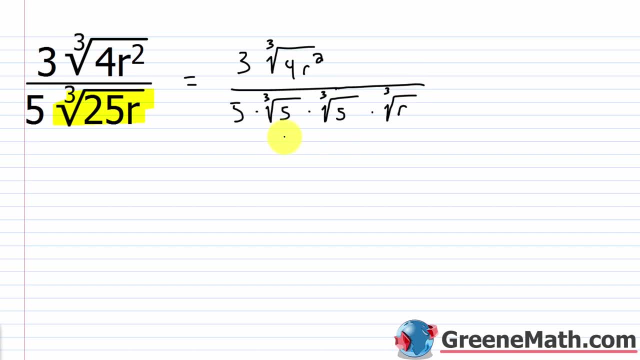 So you're thinking about how you could get a perfect cube there. You've got five times five there. You just need another five to get a perfect cube. Five times five is 25.. Five times another five would be 125.. That's a perfect cube. 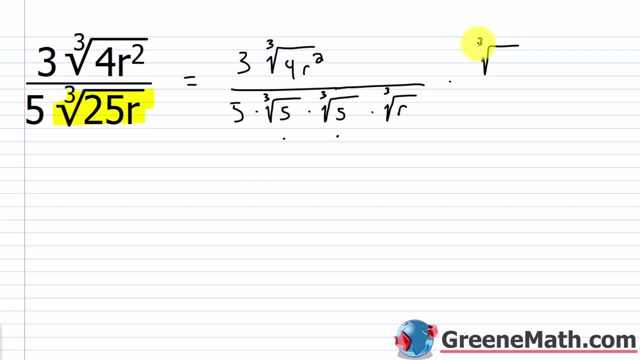 So when you do this, you want times, the cube root of five, But you also have to think about this R. here You have the cube root of R. You need to make that a perfect cube also. So if you just have R to the first power. 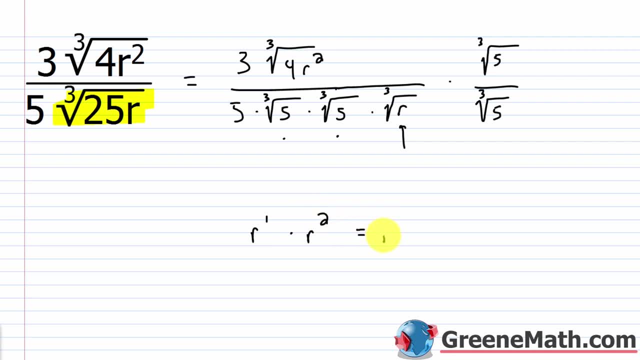 you're gonna need to multiply that by R squared so that you can get R cubed and have a perfect cube. So we would add under here R squared, and you do the same thing in the numerator and the denominator. So this is how you go about setting these things up. 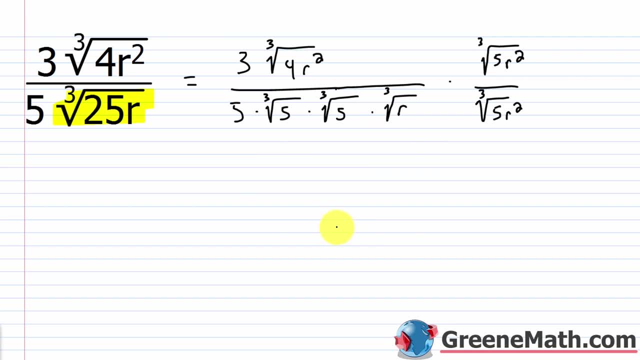 Especially when you get into these higher level roots, you wanna take the time to break things up and see what's needed. If you don't, you might end up costing yourself a lot of extra time, or you might just outright get the wrong answer. 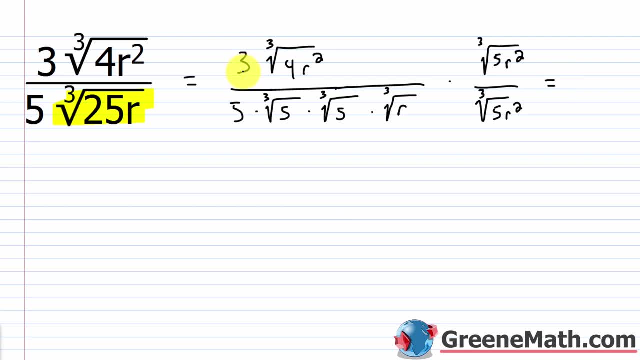 All right, so let's go through and multiply. So in the numerator we'll have three, Which is multiplied by the cube root of four R squared times the cube root of five R squared. So this would be the cube root of four times five, which is 20. 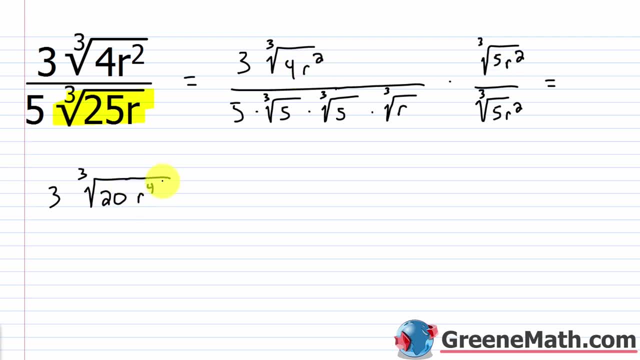 times R squared, times R squared, which is R to the fourth power. Of course we can simplify this and we'll deal with that in a second Over. we'll have five multiplied by, we'd have five times five, which is 25, times another five, which is 125.. 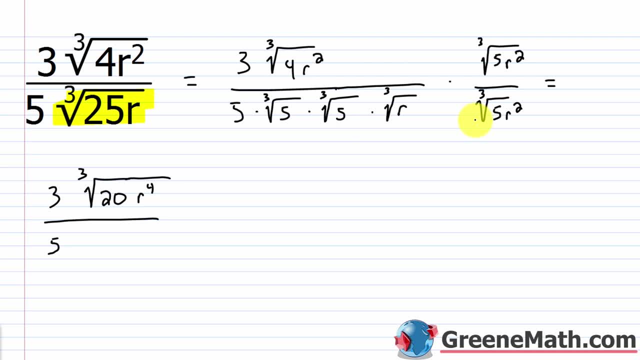 So it would be root of 125, which is 5,, so 5 times 5.. And then you'd end up with the cube, root of r, cubed, which is r. So my denominator is radical free. So in the denominator we would basically just: 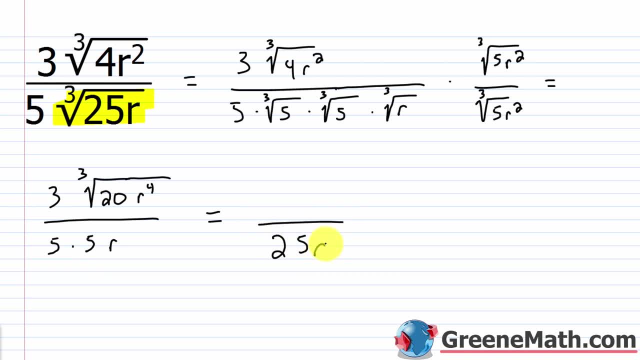 have 25r In the numerator, you'd have 3 multiplied by 20 is what It's 5 times 2 times 2.. There's no perfect cubes in there, so you can just leave that 20.. So we'll put the cube root. 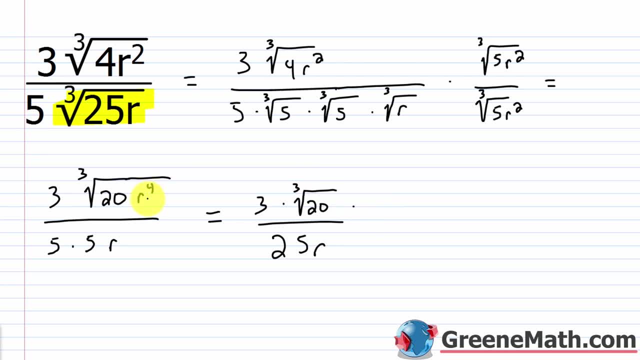 of 20 multiplied by. when we think about the cube root of r to the fourth power, we know we can simplify this Again if the exponent here is the same or greater than the index. you can simplify. You could split this up into the cube root of r, cubed multiplied by the. 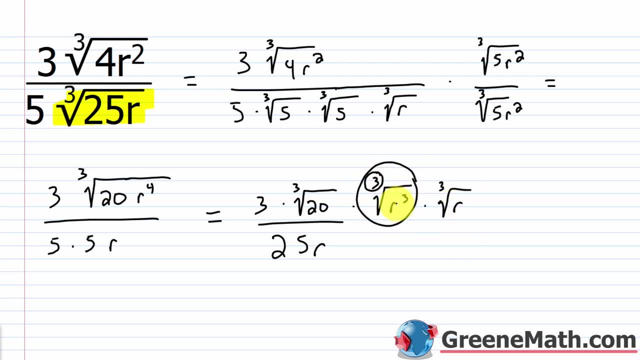 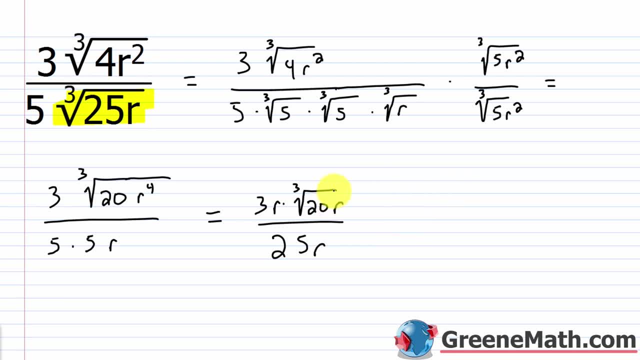 And then I can get rid of this, And then I can get rid of this, And then this r can go underneath here. Now, before I conclude, my problem, this is multiplication here. So I don't need to factor anything, I can just cancel. I can cancel common factors, This r, with this r ended up with 3 times. 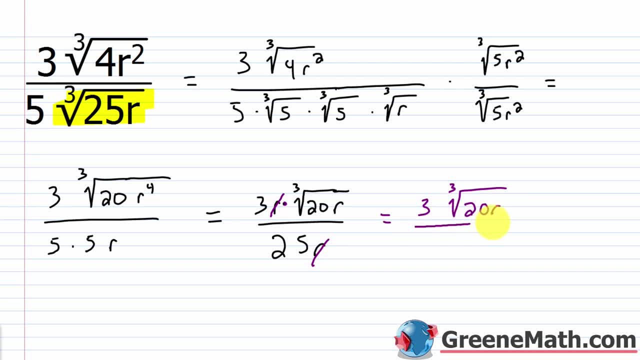 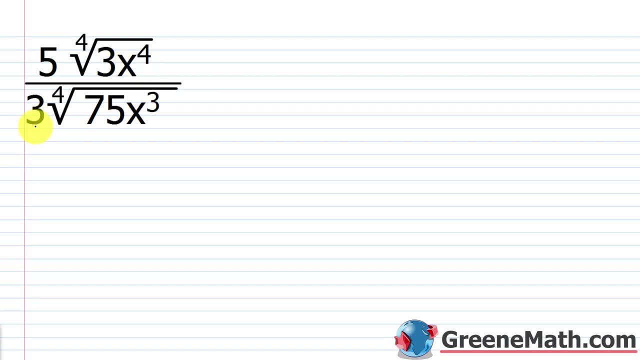 the cube root of 20r over 25.. All right for the next one. let's take a look at 5 times the fourth root of 3x to the fourth power over 3 times the fourth root of 75x cubed. 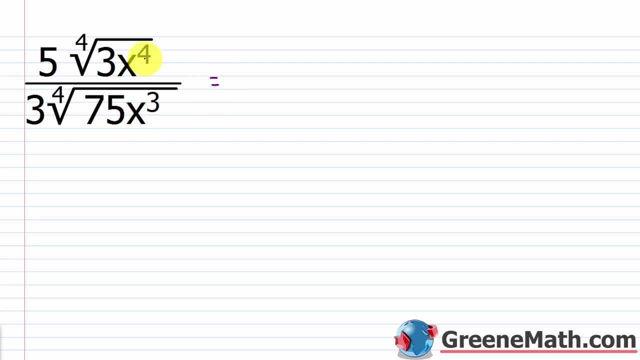 So when we look at this in the numerator, if we have x to the fourth power, we're taking the fourth root of that. We know that's just x. So we can simplify that. to start and just say I have 5x. 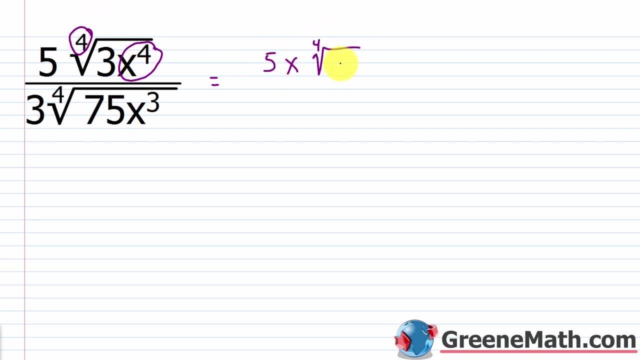 right, I just pulled this out. times the fourth root of 3.. Okay, then this is over. We have 3 multiplied by, we have the fourth root of 75x cubed. Now, x cubed is not a perfect fourth. 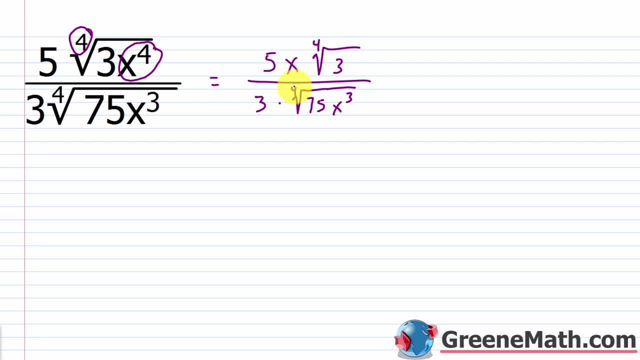 so we can't do anything about it. We can't do anything about it. We can't do anything about that. And 75 is not a perfect fourth. But again, we're going to think about what we'd need to do to get a perfect fourth. So 75 is what It's 5 times 5, which is 25, times 3.. And then x cubed. 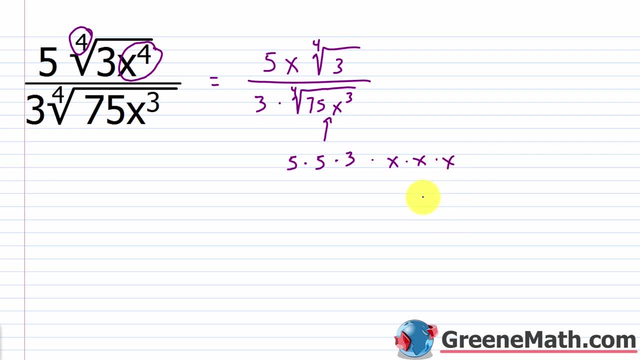 is x times x times x. So I know to get a perfect fourth here, I just need one factor of x. right, That's it. One more factor of x. we'll be good to go there For this guy. I need two factors. 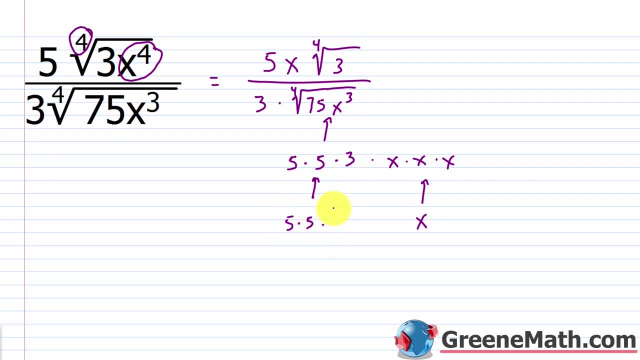 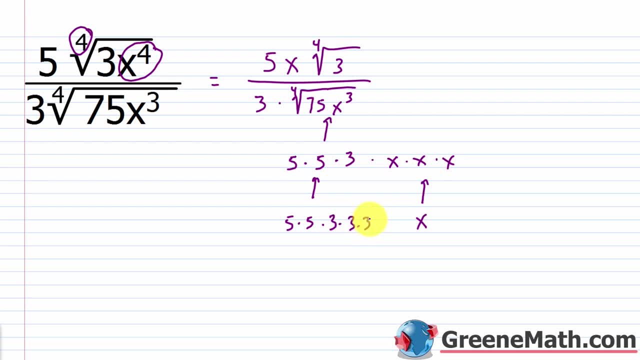 times 3 again, which is 225, times 3, one more time, which is 675.. So we'll need to multiply this by the fourth root of 675, and then x. Okay, we'll do that to the numerator and denominator. 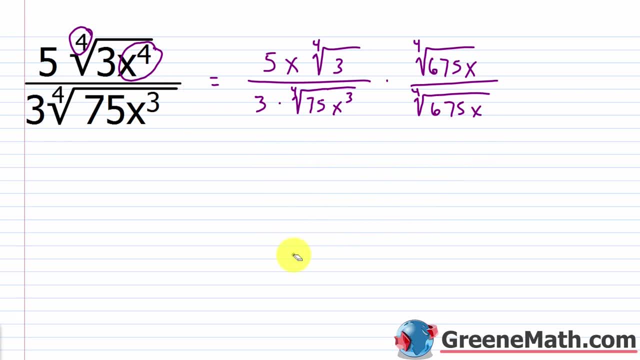 All right, let's erase this and let's crank this out. So we'll have 5x multiplied by the fourth root of 3, times the fourth root of 675x. over, you'll have 3 multiplied by the fourth root of 75x cubed times the fourth root of 675x. 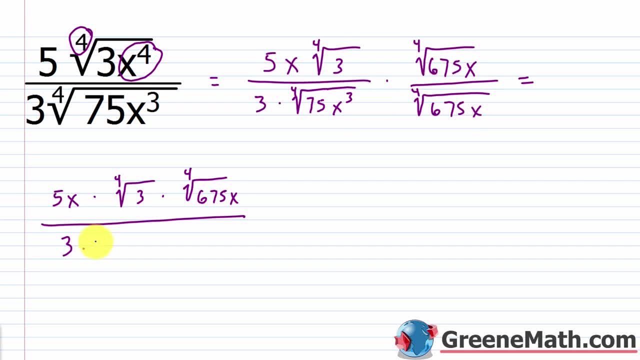 We know the fourth root of x to the fourth power would just be x, So let's just do that first. 75 times 675 ends up being 50,625.. But we don't need to think about that, because we built this by looking at the prime factors. We remember it was 5 times 5 times 3 to get to 75.. So I only used 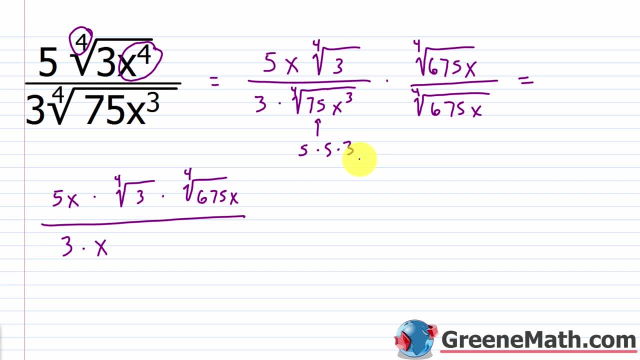 two prime numbers. in this I used a 5 and a 3.. So basically, this number that we end up with is 5 to the fourth power, times 3 to the fourth power, Or in other words, it's 15 to the fourth. 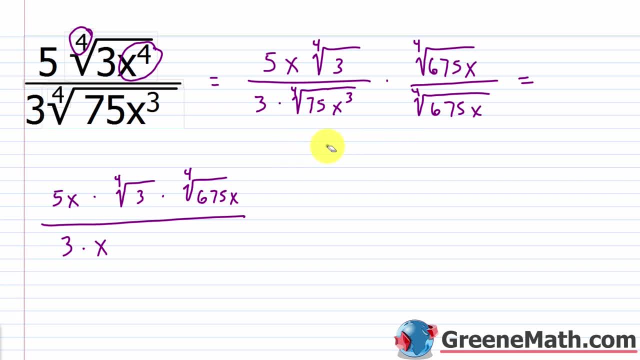 power. So the fourth root of 15 to the fourth power is just 15.. So times 15.. 3 times 15 is 45. So let's write this as 45x. Now, before we do anything else, we notice that 5 would cancel. 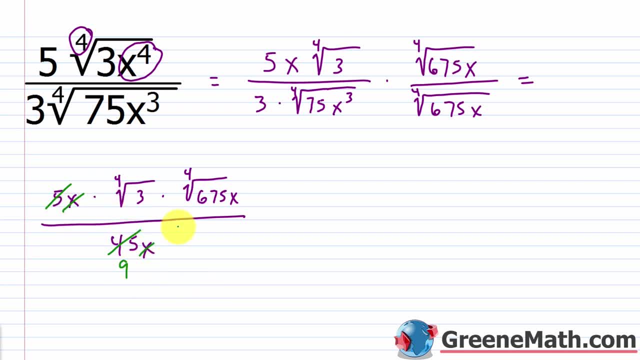 with 45.. This would be a 9.. And x would cancel with x. Now, what are we left with now? If we look at the numerator, we've got the fourth root of 3 multiplied by the fourth root of 675x. 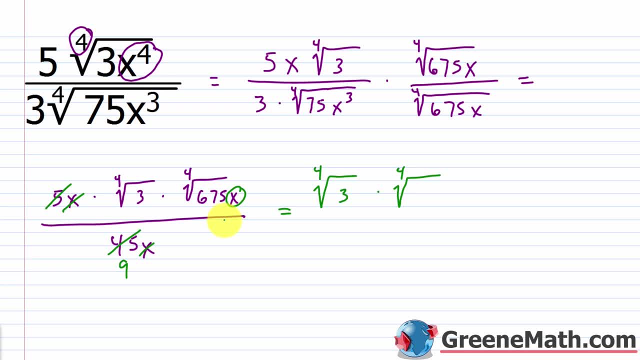 So we know we're not going to be able to do anything with this, But when we think about 675, that came from two factors of 5, or 25.. And it came from three factors of 3, or 27.. 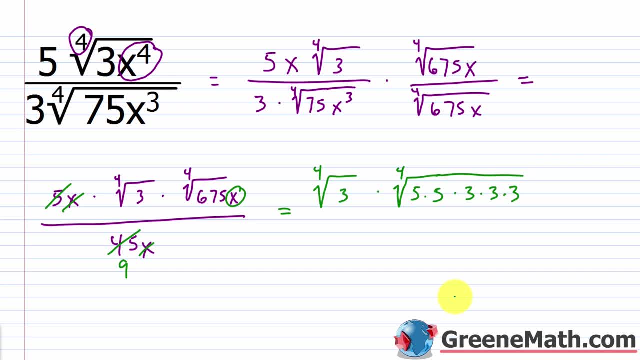 So we look through here and we look for a perfect fourth- Let me put times- the fourth root of x, just so we don't forget that. So we would have what 1, 2,, 3,, 4 factors of 3, or 81.? 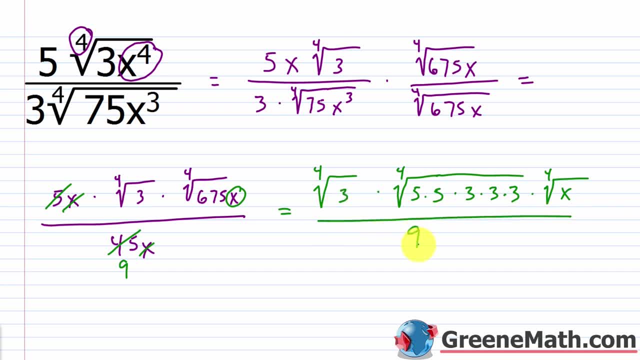 Let me just complete this. I'm going to put over 9.. So you would have the fourth root of 81 times the fourth root of 5 times 5, or 25, times the fourth root of x over 9.. This right here has a. 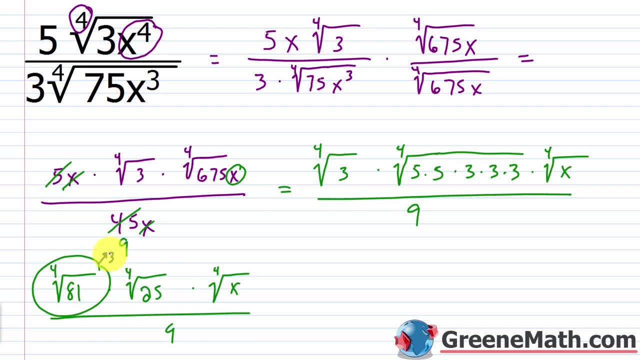 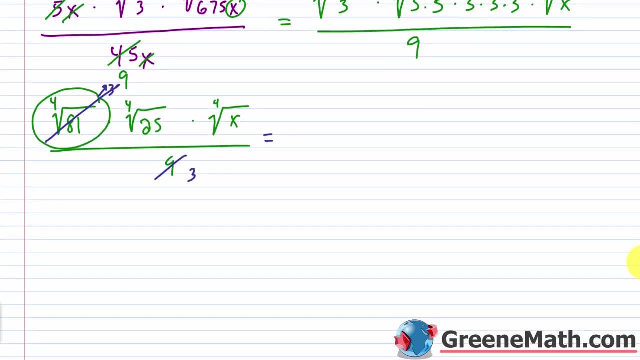 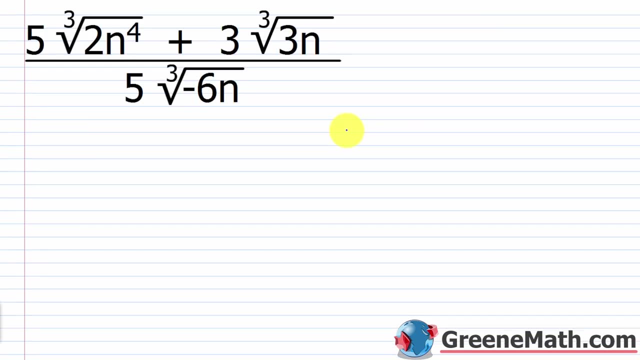 value of 3.. So you basically have a 3 here. So I could cancel this with this and leave a 3.. And as my answer is going to go, we would end up with the fourth root of 25x over 3.. All right, so for the next one we have 5 times the cube root of 2n to the fourth. 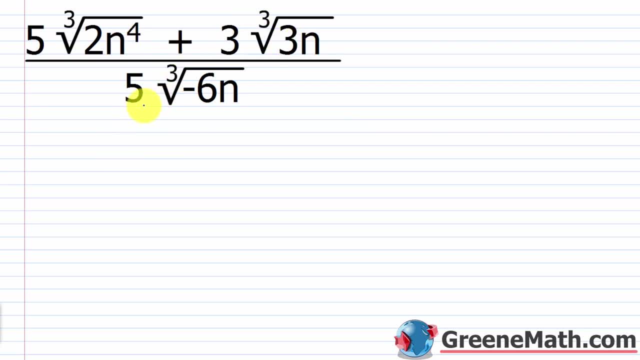 power plus 3 times the cube root of 3n, over 5 times the cube root of negative 6n. So what we want to think about here we have 5 times. let's break this up a little bit. We know if we see an. 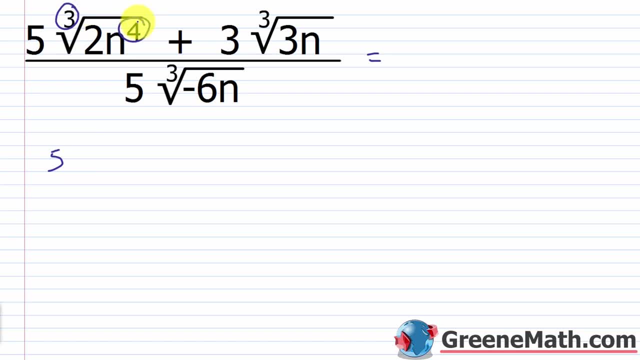 index of 3 and an exponent of 4, we can do something there. So let's say we have the cube root of 2 n cubed times the cube root of just n, plus 3 times the cube root of 3n. over we have 5 times. 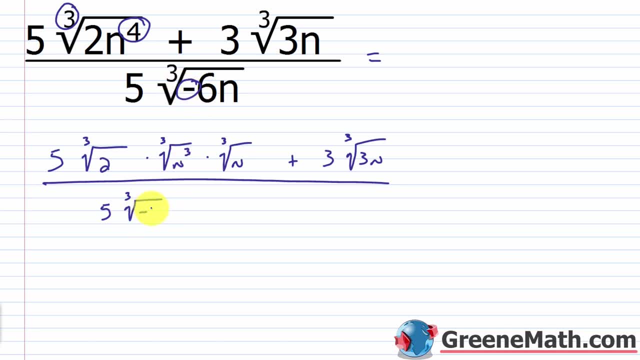 the cube root of. I'm going to split this up into negative: 1, times the cube root of 6n. This can be simplified and this can be simplified. So what we want to do, we'll have 5 times the cube root of. 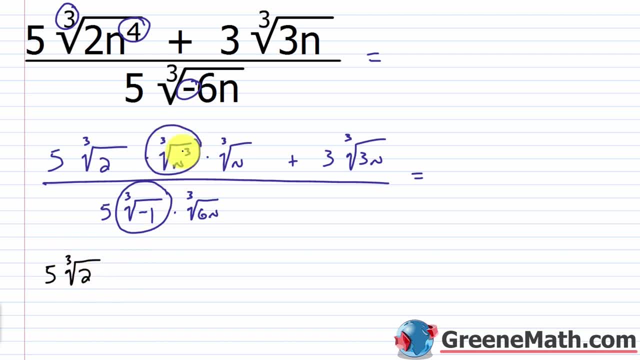 2,. this would end up being what? This would end up being, just n. So I can just write this n out in front. I'm just going to slide this down a little bit And then times you'll have the cube root of. 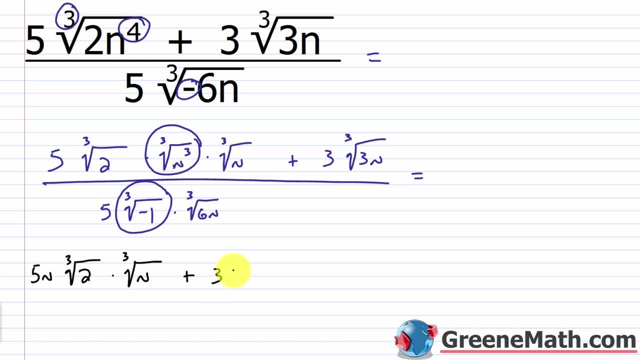 n and then plus you have 3 times the cube root of 3n and then over. this again can be simplified. The cube root of negative 1 is just negative 1.. So I'd put negative 5 out here times the cube. 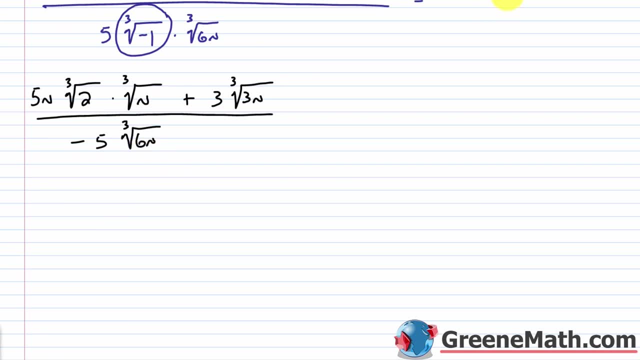 root of 6n And then plus you have 3 times the cube root of 3n, and then over. this again can be simplified. So what we want to do, we think about 6.. 6 is 2 times 3.. So really I'm not going to get. 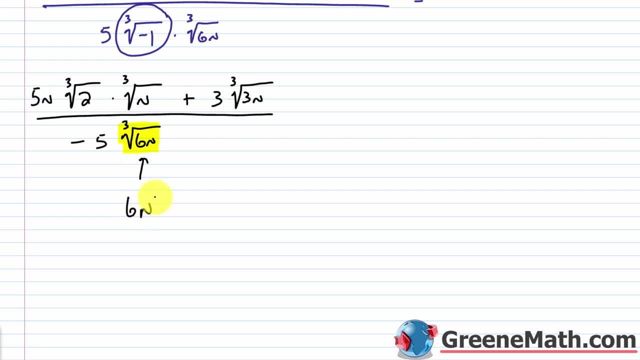 it any more simple: n is just n. So if I have 6n, all I'd want to do is multiply this by 6n. that amount squared, or 36n squared, That would give me a perfect cube. It would give me 216n. 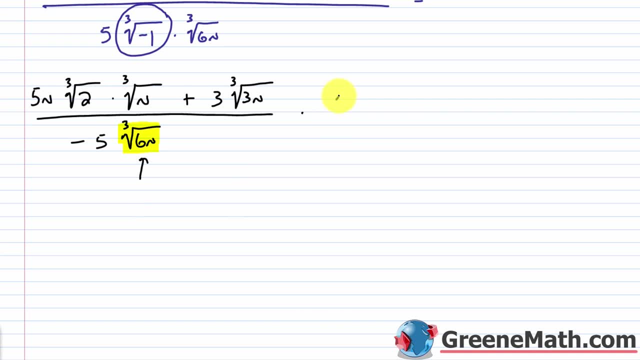 cubed, which is a perfect cube. So we'd multiply the numerator by the cube root of 36n squared and the denominator by the cube root of 36n squared, And what are we going to get Again? if I kind of combine this to make it a little easier, put this n underneath. 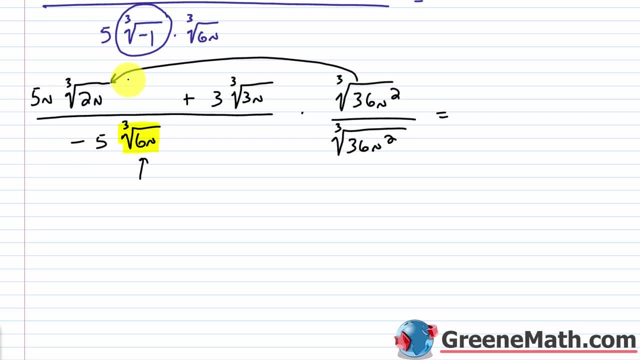 then this would get multiplied by this, So you'd have 5n out in front multiplied by the cube, root of 2n times 36n squared, 36 times 2 is 72.. n times n squared is n cubed. Then, plus This is going to multiply by this now, So you'd have 3 out in front, The cube. 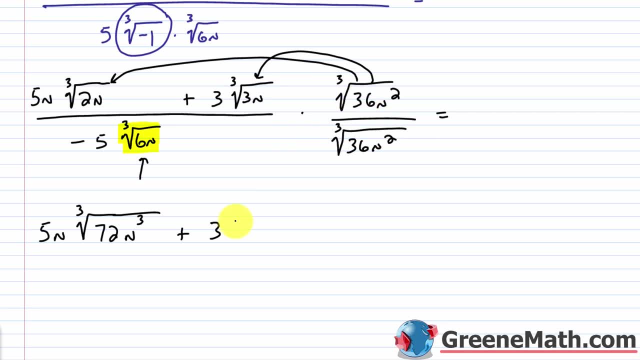 root of 3n times the cube root of 36n squared, You would have: the cube root 3 times 36 is 108.. n times n squared is n cubed. All right, then. this is over Down here you're going to have: 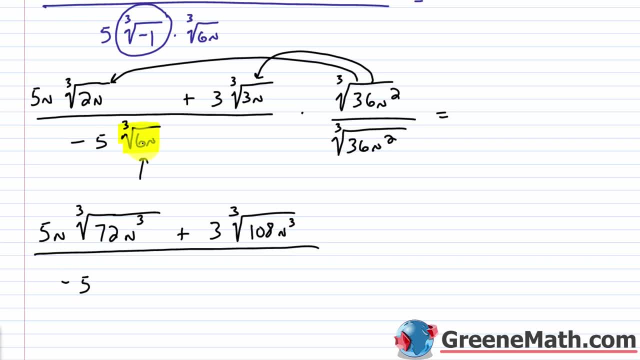 negative 5 out in front. And again, the cube root of 6n times the cube root of 36n squared is going to give you what It would be: the cube root of 216n cubed, which would basically be 6n. 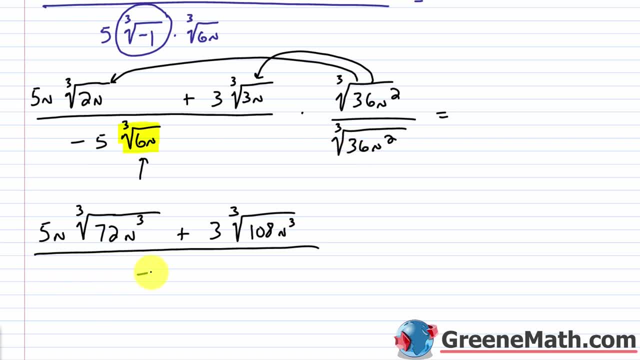 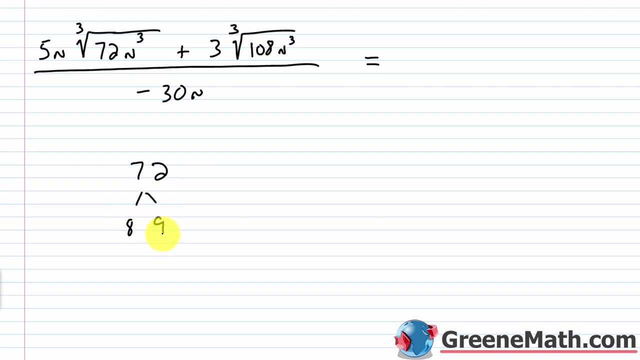 So negative 5 times 6n would be negative 30n, And now we're just looking to see can we simplify anything further. So before we try to factor anything in the numerator, let's think about 72 for a second. 72 is what It's 8 times 9.. We know 8 is a perfect cube. It's 2 times 2 times 2.. 9 is 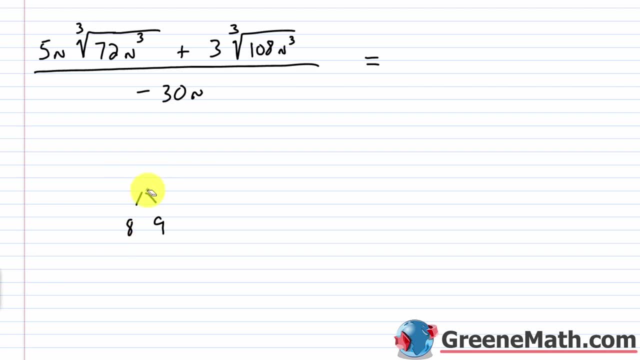 not, It's 72.. It's 2 times 2 times 2.. So we're going to try to factor anything in the numerator 3 times 3.. So what we could do is we could write this as 5n times the cube, root of 8 times the cube. 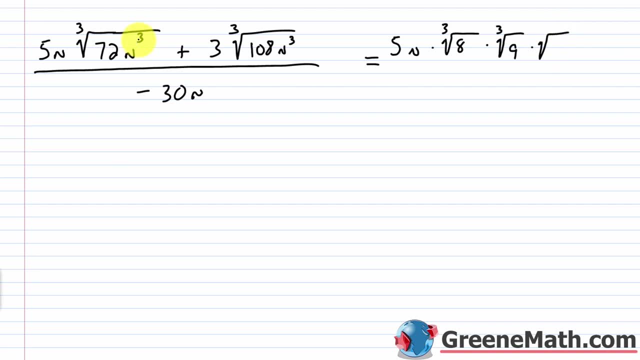 root of 9 times the cube root. When we think about this right here, this n cubed the cube root of n cubed, So these two can be simplified. The cube root of n cubed is n, So we can just make this. 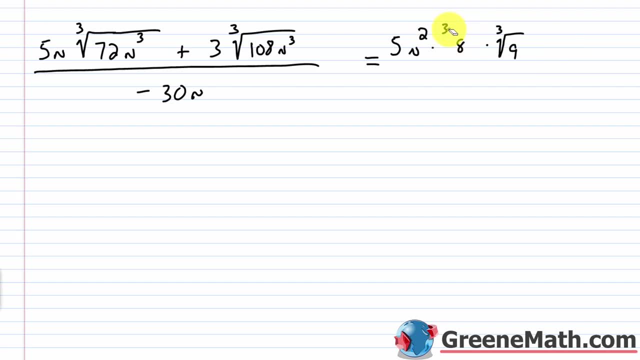 n squared, And the cube root of 8 is 2.. So we can just make this 10.. So we get 10n squared times the cube root of 9.. Then you're going to have plus Over. here we think about 108. Now what is 108?? It's divisible by 2.. It's also divisible by 3.. So we know it's. 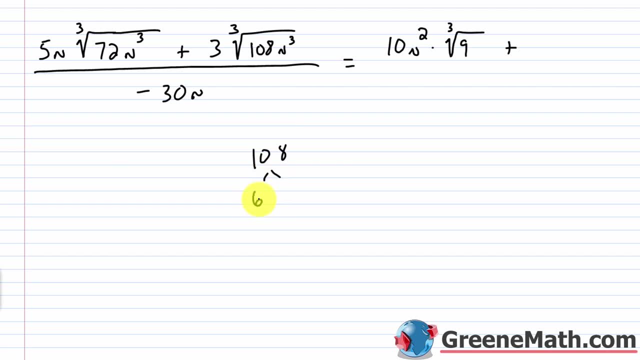 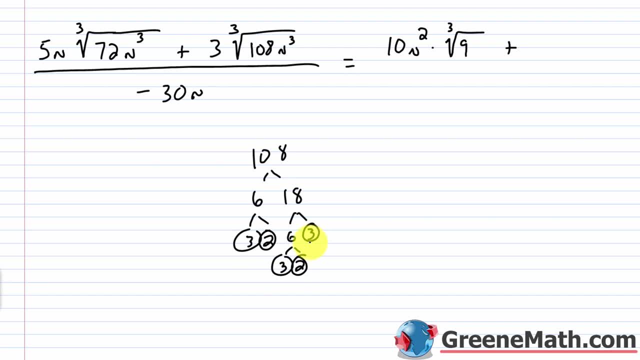 6 is 3 times 2.. You've got 1, 2,, 3 factors of 3 and 2 factors of 2.. So it's essentially 27,, which is a perfect cube times 4. So we can say this is 3 times the cube root of. let's just go. 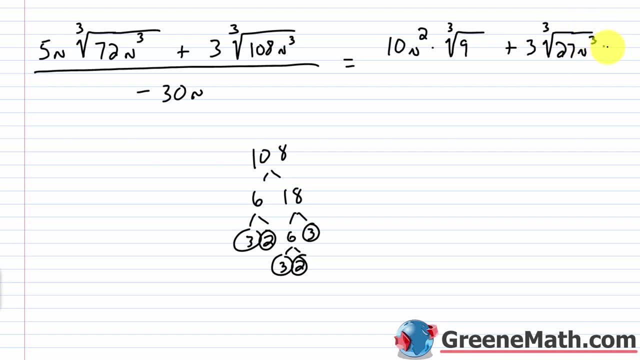 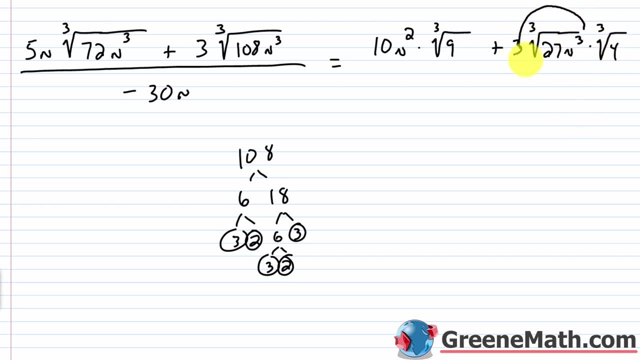 ahead and do 27 n cubed times, you'd have the cube root of 4.. Now again, this part right here can be simplified. The cube root of 27 n cubed is going to be 3n. So 3n multiplied by this 3, that's already here. 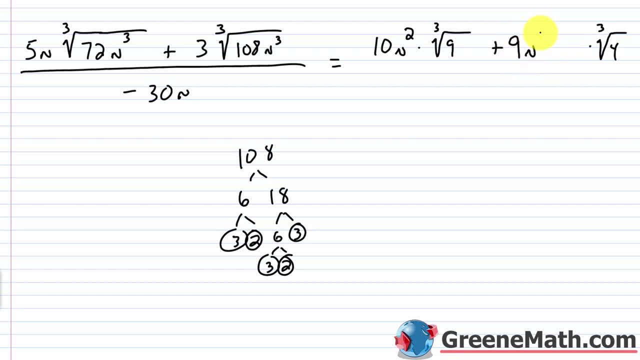 would give us 9n. So this would be 9n multiplied by the cube root of 4.. Then over we'll have negative 30n. Now here's the question Again, because this is addition. can I factor anything out and then cancel? Well, number-wise, the answer to that is going to be no. 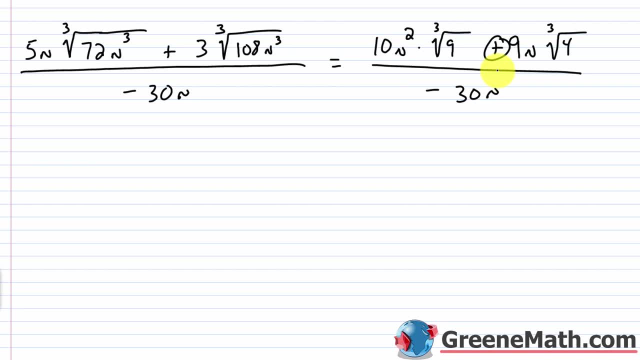 10 is 5 times 2.. 9 is 3 times 3.. Nothing I can really do there But variable-wise. yes, I have n squared and I have n, So I could factor an n out and I'd have 10n times the cube root of 9 plus 9. 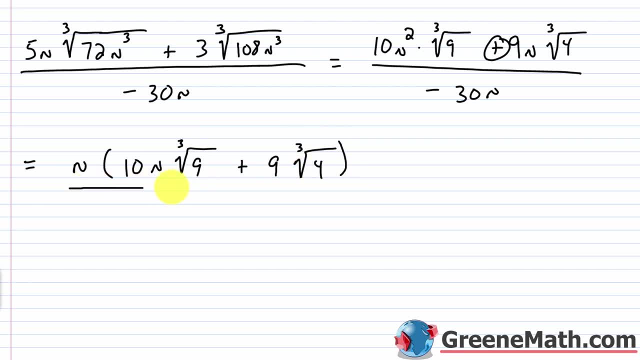 times the cube root of 4 over negative 30n, Then this would cancel with this And what I'm left with we'd have 10n If I'd taken maybe the integral instead of this, the 15th over peri-ametrist. if I hadn't done that, I wasn't actually 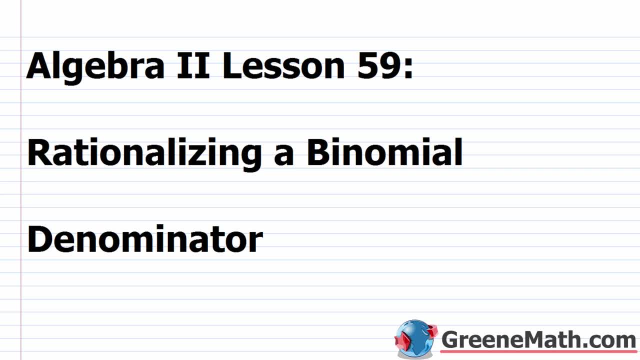 Then we'd have depressed the 5th being 3n divider over pi divided by 4.. Then now we could say, yeah, this is a 10 to the power. So I've got a root and I've got a negative Treat: 2 through negative 34 plus 5.. 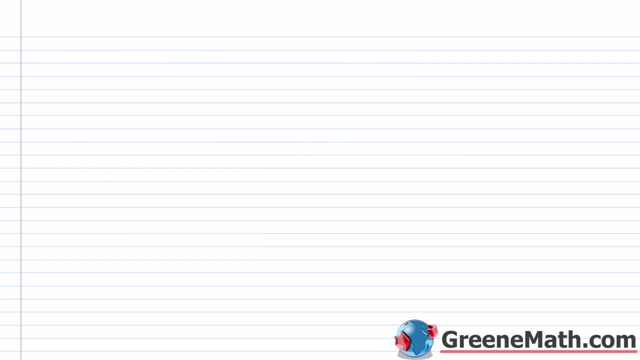 He gave me my 3 over here, as the integral was nothing but 50. All right, Then we'd have negative 24 times that 4 over 9, plus 9. Times the cube root of 9.. Plus 9 times the cube root of 4.. 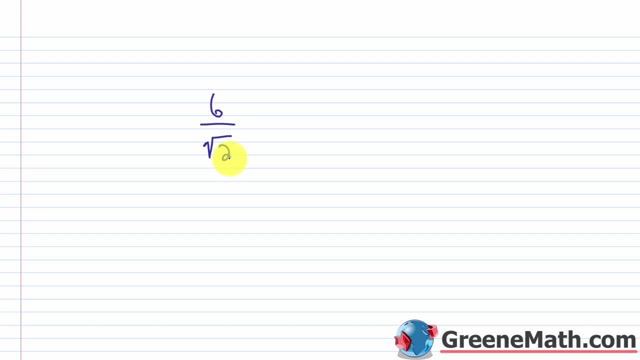 And then this is over. We'd have negative 30. 2.. So we should all know at this point, if we see this, this is not considered simplified, because the rules tell us that we don't want a radical in the denominator. Now, depending. 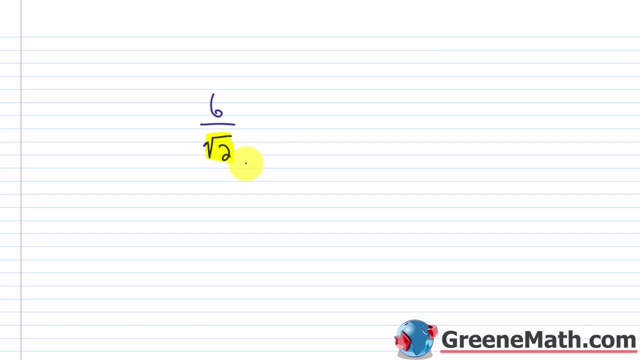 on what you get. you might get a square root in the denominator cube root, fourth root, fifth root, whatever it is, you need to apply a little trick. So with this guy right here, since it's a square root, I'm just looking to multiply by the square root of 2 and I'm 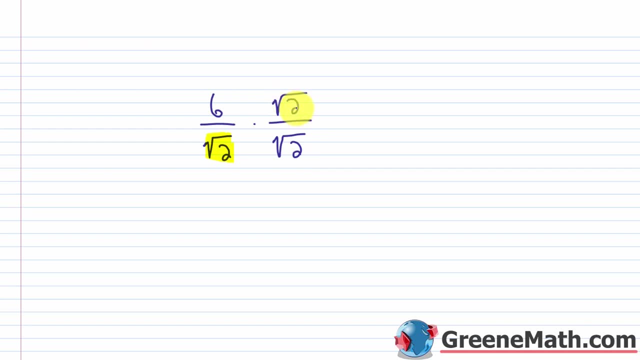 going to do that to the numerator and the denominator. That's what makes it legal right. Square root of 2 over square root of 2 is 1, multiply by 1. you leave something unchanged. When we do this, we will be radical free in the denominator: Square root of 2 times square. 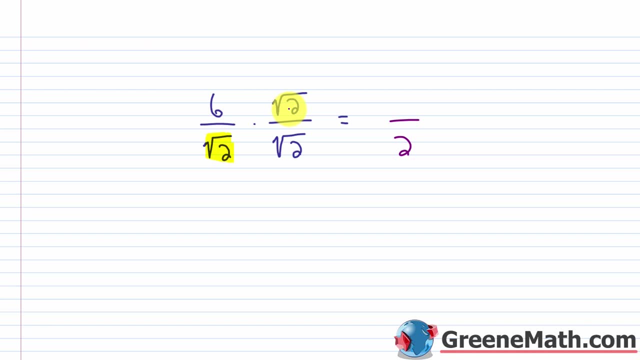 root of 2 is 2.. 6 times square root of 2 is just 6 times the square root of 2, and of course we can simplify this further: 6 divided by 2 is 3.. So this would end up giving us 3 times. 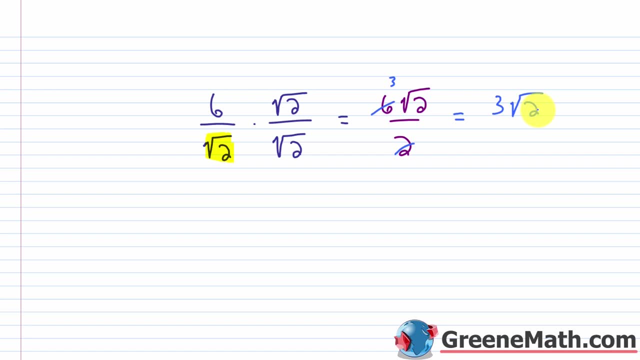 the square root of 2.. But the main idea here is just to understand that this right here is considered simplified and it is preferred to this right here. They are the same value, they are equal to each other, But it's just like when we saw something. 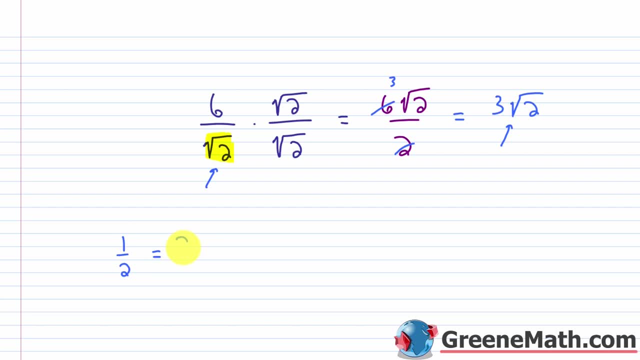 like 1 half and 2 fourths. Mathematically, in decimal form, these are both .5.. But we prefer 1 half to 2 fourths. right, 1 half is considered simplified and it's the same thing with this scenario here. 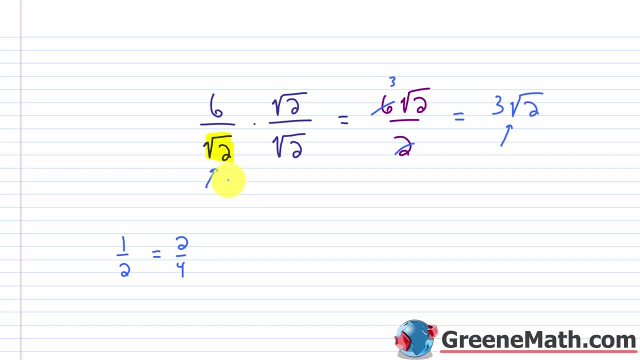 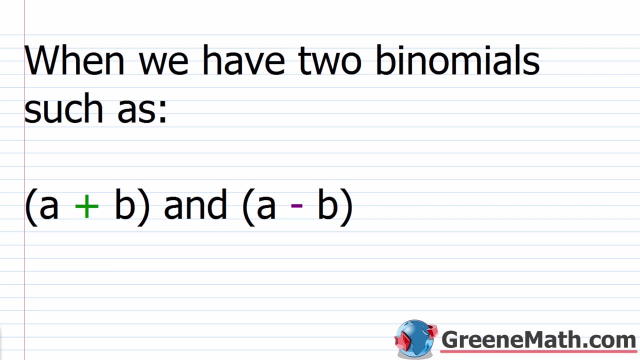 Now in this lesson we're going to look at some more complex scenarios. The first thing we're going to do before we jump into that, we need a little back story here. So we're going to backtrack a little bit, we're going to learn a definition and 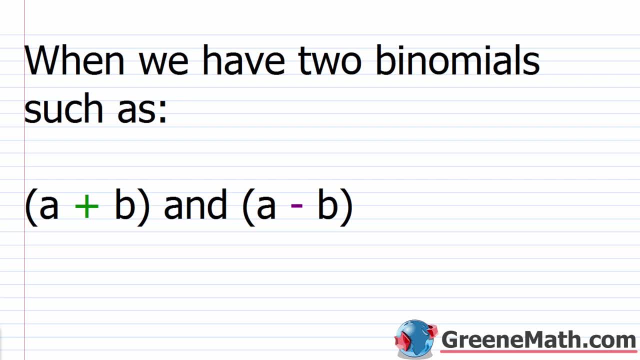 then we're going to move ourselves forward, And I'm going to show you how to do this. when you have two terms in the denominator, So when we have two binomials, such as A plus B and A minus B, if the first terms are identical and the last terms are identical, and only 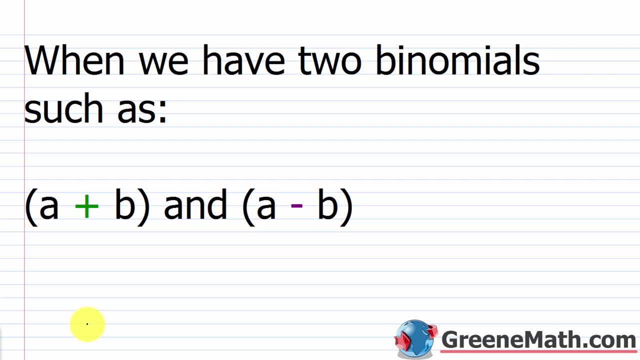 the signs did it. then the term is correct. As you can see, those terms both kind of differ. you have conjugates, Okay, so here you have A and you have A, here you have B and you have B. and then your signs are different. You have a positive and you have a negative. 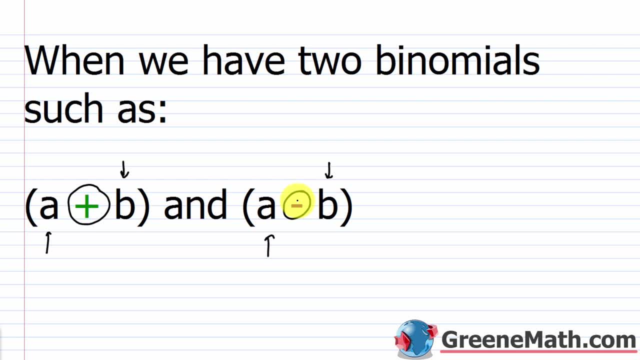 You'll recall that we already worked with these before. we just didn't refer to them as conjugates at the time. When you multiply the two together using FOIL, the outer and the inner cancel each other out, and so you're just left with the first term squared minus the last term squared. 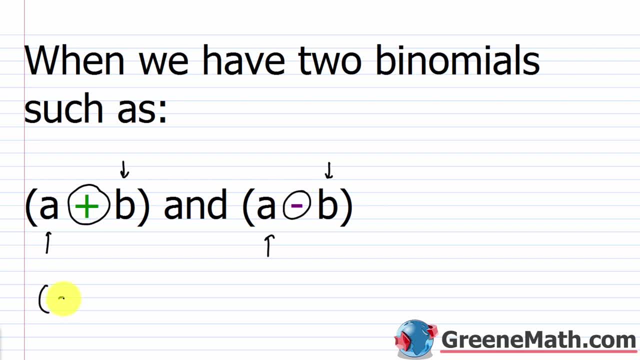 right, We call it the difference of two squares. So if I had something like A plus B multiplied by A minus B, you could do this the long way. A times A is A squared. The outer A times negative B is minus AV. The inner B times A would be plus BA or plus AV, however you want to write that. 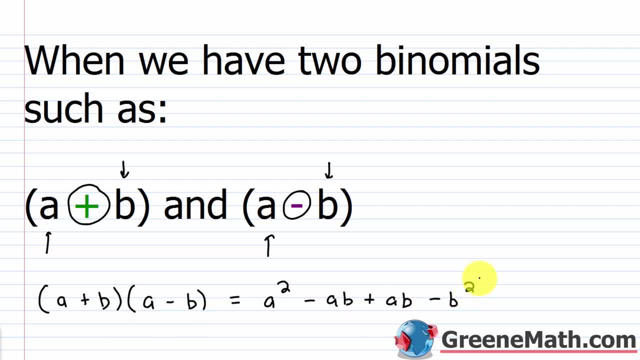 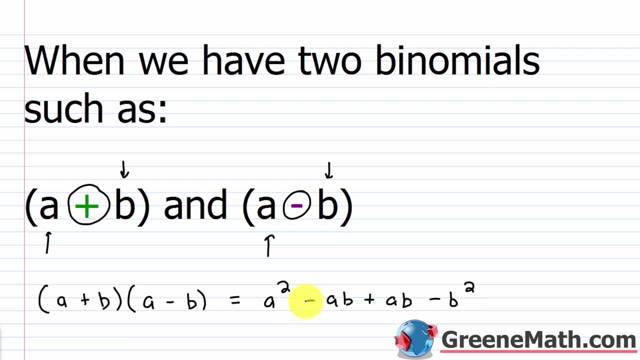 So again this becomes the difference of two squares. You see that these two would cancel each other. The outer and the inner terms cancel each other and you're left with the first term squared, so you've got A squared, minus the last term squared, so you've got minus B squared there. 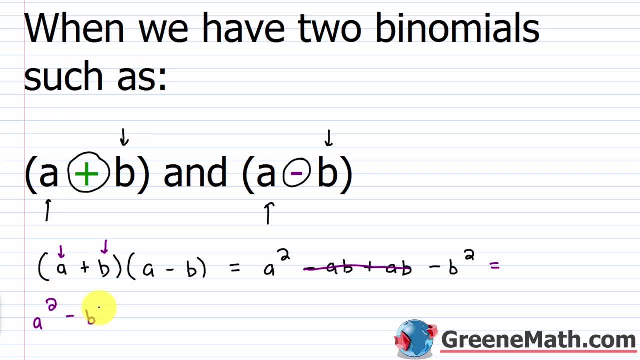 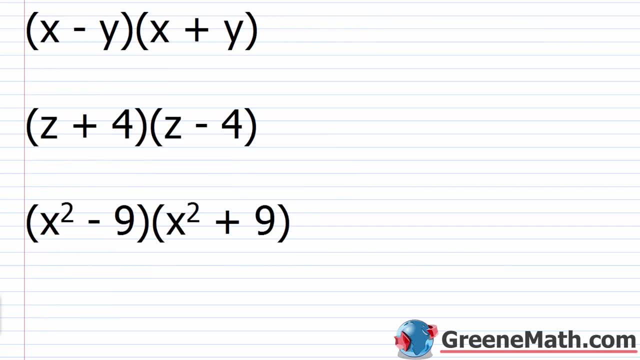 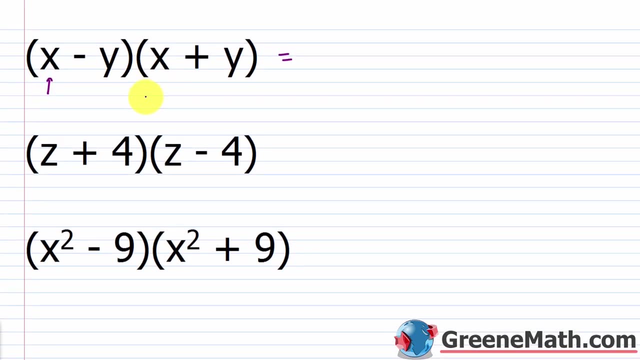 So we put equals A squared minus B squared, And we know this from working with special products. So let's look at some quick examples. So, without doing FOIL, we already know that if we have X minus Y times X plus Y, it's Y Again. I've got X here and here. I've got Y here and here. 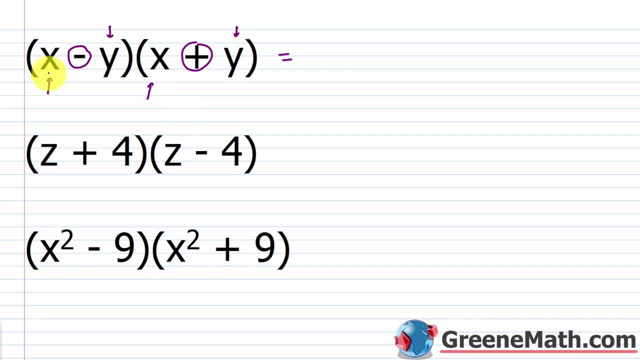 I've got different sides, I've got a minus and I've got a plus. So I would just say this is X squared, the first guy squared minus the last guy squared, which is Y squared, the difference of two squares. For this guy, we have Z plus 4 times Z minus 4.. So again, if I multiply this out, I get Z squared. 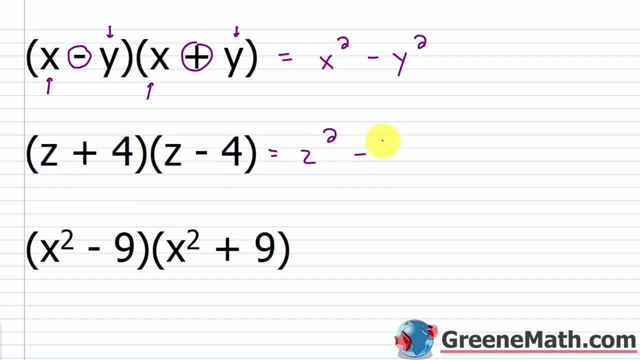 the first guy squared minus 4 squared. The last guy squared. Now you can write 4 squared or you can just write 16, because we know 4 squared is 16.. All right, so we look at X squared minus 9 times X squared plus 9.. Again, this would be X squared. 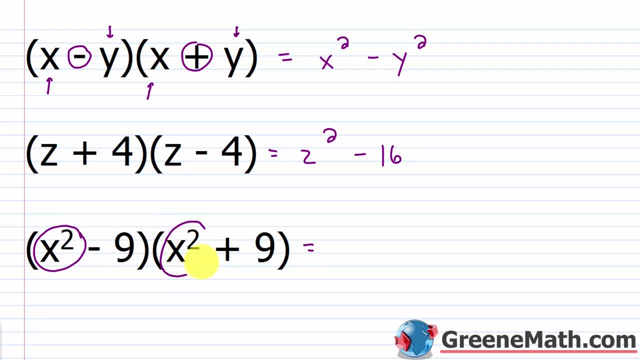 squared right. This is what we have here in the first position of each. So it's X squared squared. All right, just think about, if I multiply X squared times X squared, That would be what X to the fourth power, or X squared squared. 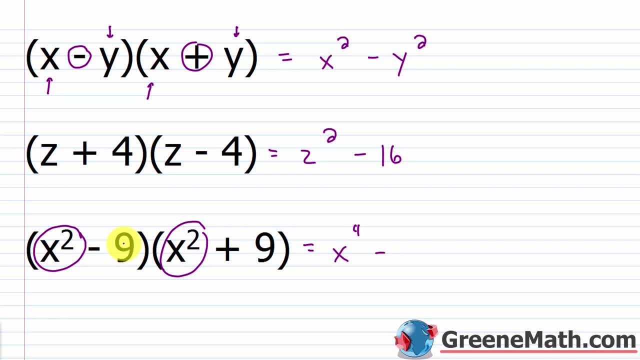 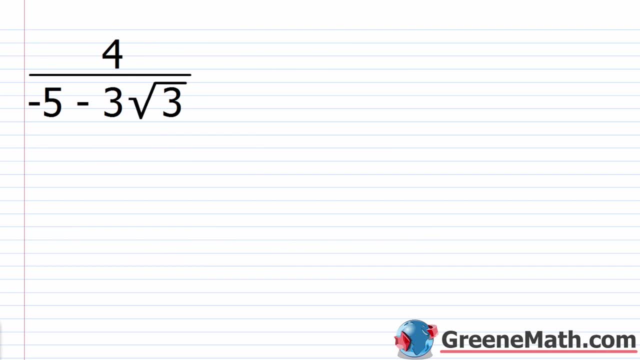 Then minus this guy, squared 9, squared is 81.. All right, so let's apply this knowledge And let's look at an example here. So suppose you see 4 over negative, 5 minus 3 times the square root of 3.. 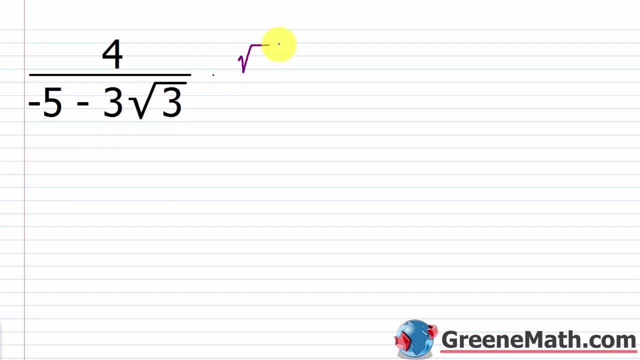 You can't just do this times square root of 3 over square root of 3, like we've been doing. That's not going to leave you radical free in the denominator. What you need to do is multiply the numerator and denominator. What you need to do is multiply the numerator and denominator. What you need to do is multiply the numerator and denominator. 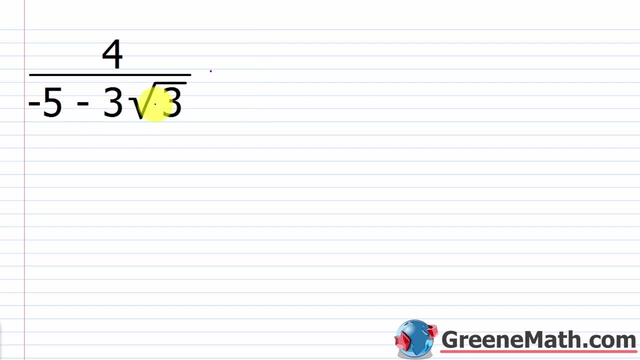 By the conjugate of the denominator. So what is the conjugate going to be? Again, the first terms would be the same. So I have a negative 5 here. So for the conjugate I'd have a negative 5.. The signs will be different. That's a minus, This would be plus. 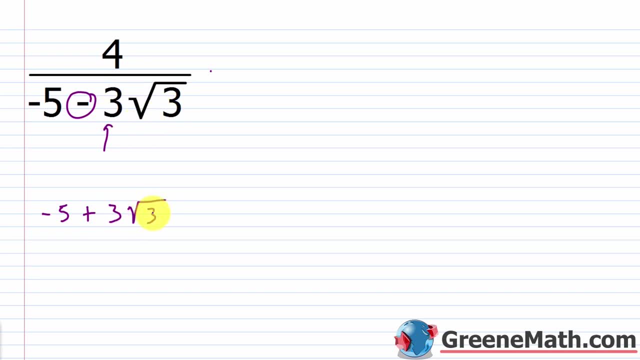 And then this guy would be the same 3 times square root of 3.. So these two would be conjugates, okay? So what I'm going to do? I'm going to multiply by negative 5 plus 3 times square root of 3. 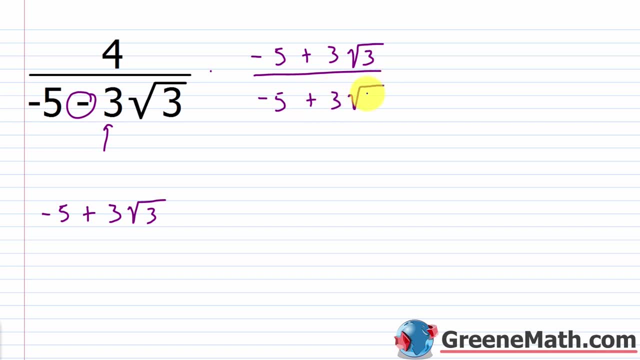 over negative 5 plus 3 times square root of 3.. And I know some of you don't believe this, but it's going to end up leaving you with a radical free denominator, All right, so let's take a look And you just think about this. putting parentheses around this, 4 would get multiplied by negative 5,. 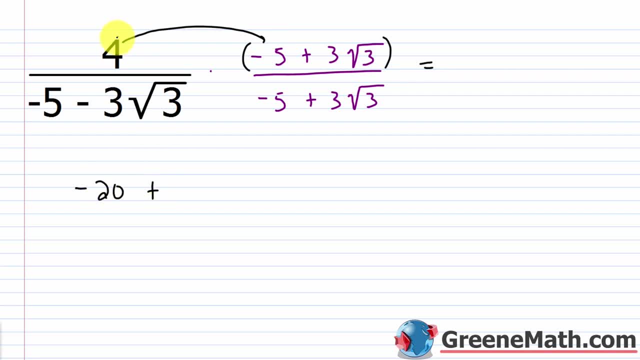 which would give us negative 20.. And then plus 4 would get multiplied by 3 times the square root of 3.. 4 times 3 is 12.. So you'd have 12 times the square root of 3 there, Then down here: 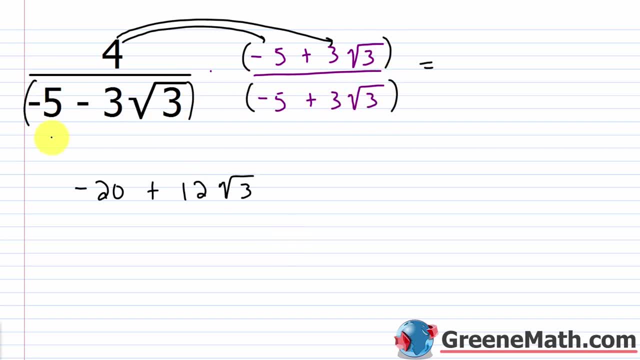 you basically think about this as using FOIL, But again, because this is something we know already, the outer and the inner they're going to cancel. All right, I would do negative 5 times negative 5, that would give us 25.. The outer: negative 5 times, 3 times the square root of 3,. 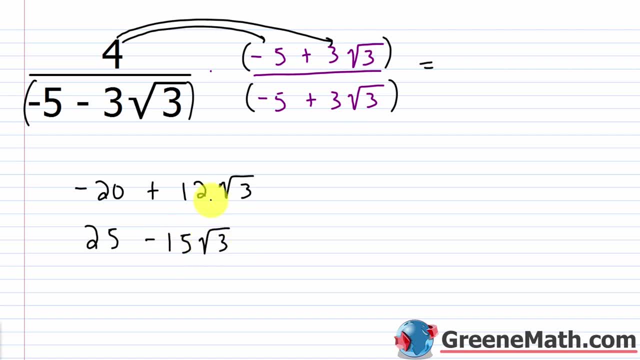 would be negative 15 times the square root of 3.. The inner negative 3 times square root of 3. times negative: 5, would be positive 15 times square root of 3.. And then negative 3 times square root of 3. times positive: 3 times square root of 3, would be negative 9.. And then: 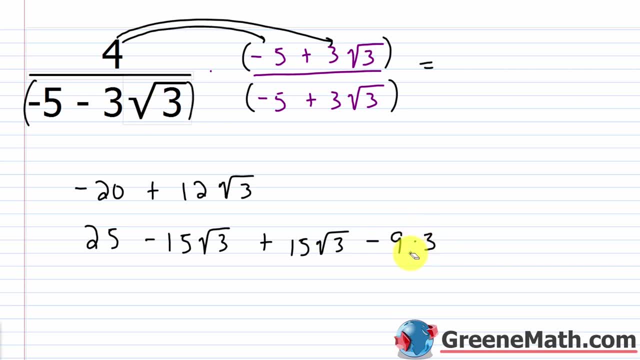 square root of 3 times square root of 3 is 3, so times 3.. So this is basically negative 27.. Now again, the outer and the inner are going to cancel. These are opposites. those are gone. 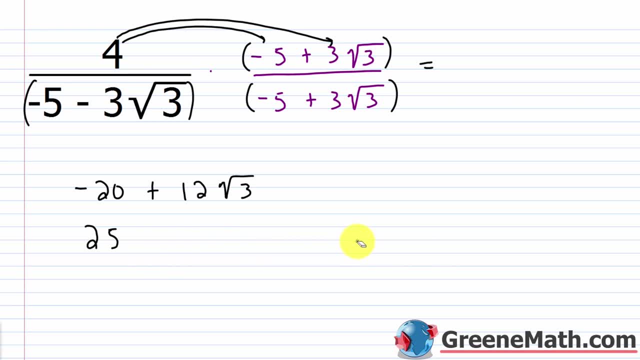 So you're left with 25 minus 27.. And what does that give you? It's going to give you negative 2.. In the numerator we have negative 20 plus 12 times the square root of 3. So I'm radical free. 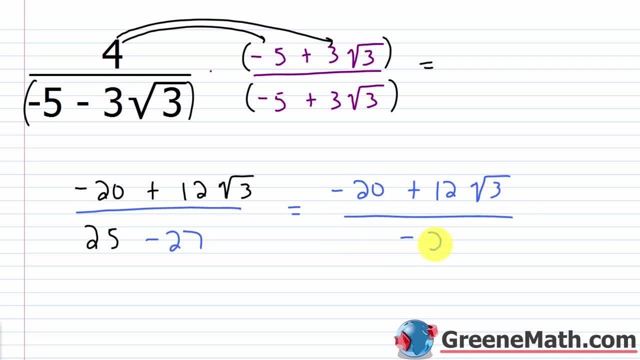 in my denominator. now, I'm not done simplifying, but I am radical free. Now what else can we do? Well, one thing is, a lot of people don't like having a negative in the denominator, So you could factor out not only a 2, but a negative 2 from the numerator. So let's go ahead and do. 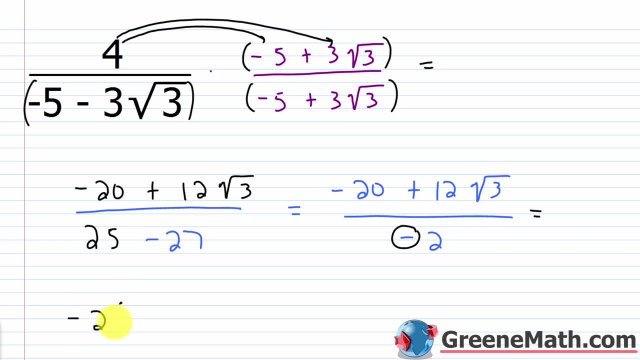 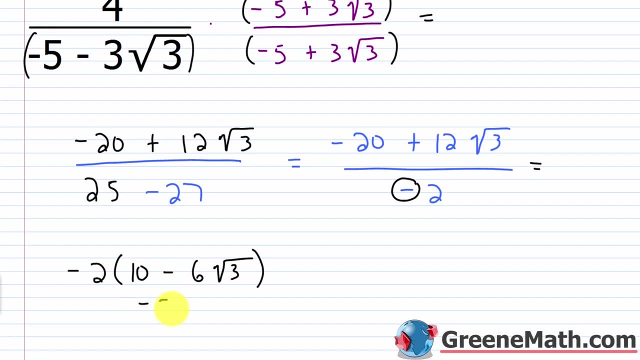 that If we factored out a negative 2, we'd have a negative 2 out in front And then, inside of parentheses, we'd have a positive 10 minus 6 times the square root of 3.. And this is over negative 2.. So what's going to happen is we're going to cancel this negative 2. 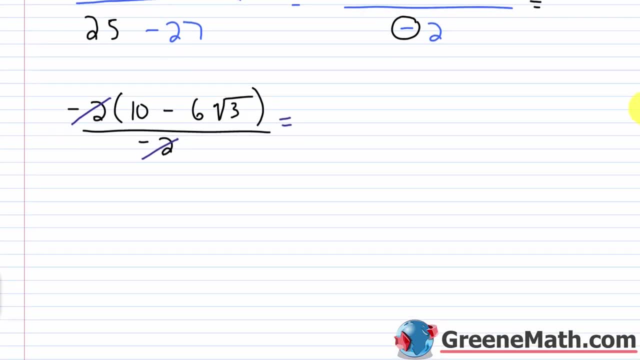 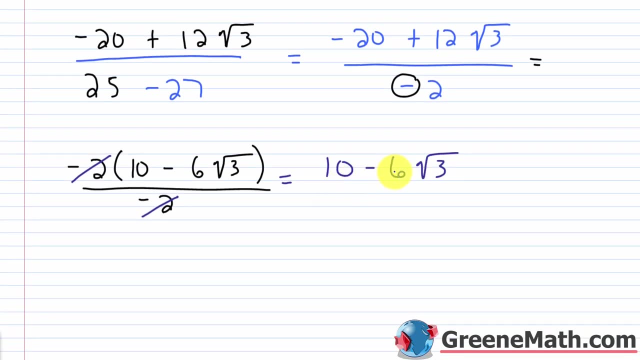 with this negative 2. And we're left with our answer here. So this is going to simplify into 10 minus 6 times the square root of 3.. Now, nothing else I can do to make that any simpler. Let's take a look at another one Again. once you kind of get used to these, they're very 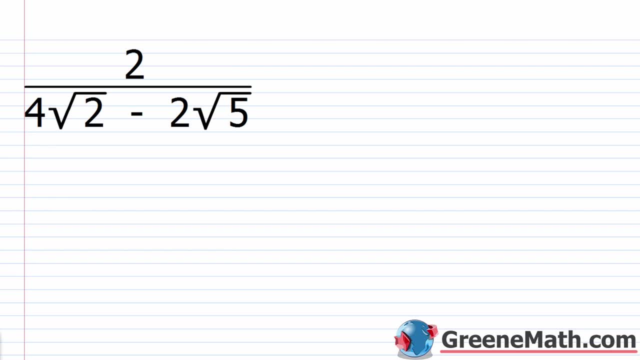 very easy, Not any more Difficult. It is a little bit more work because of the simplification, But again, it's conceptually not any more difficult. So we have 2 over 4 times the square root of 2, minus 2 times the square root of 5.. 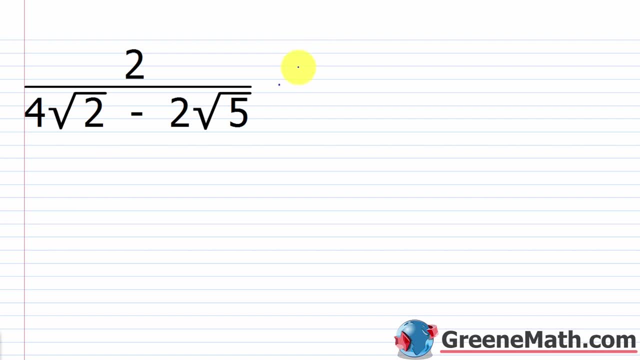 So again, all I want to do is I want to multiply the numerator and denominator by the conjugate of the denominator. So this will be the same and this will be the same. We just have to change the sign. So we would have 4 times the square root of 2.. Instead of minus, we're going. 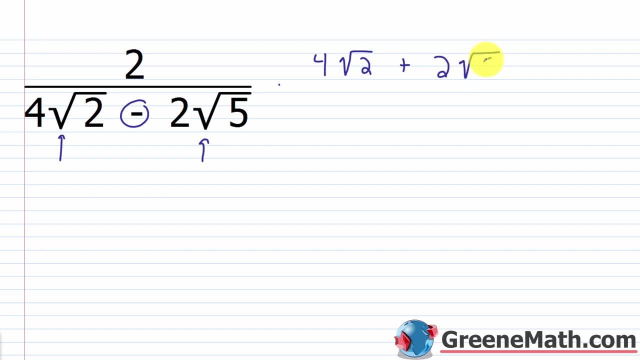 We're going to have a plus and then 2 times square root of 5.. We do the same thing for the denominator and we're going to multiply. So 2 times 4 times square root of 2 would be what. 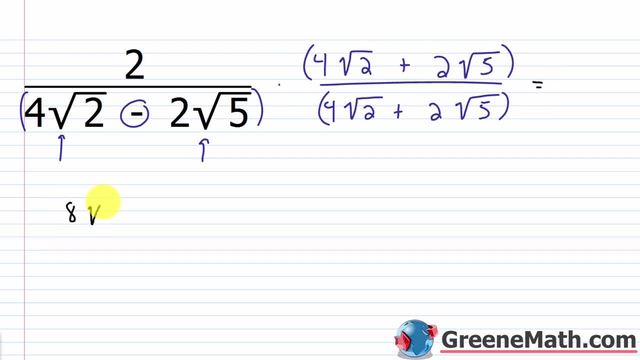 This would give us 8 times square root of 2.. Then plus, if we have 2 times 2 times square root of 5, 2 times 2 is 4, then times square root of 5.. And then this is over. 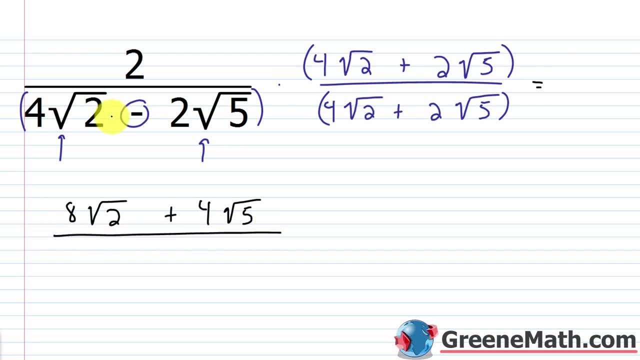 Down here again. let's use our shortcut. Let's not go through and use FOIL. We know it would be the first guy squared. So if I square 4, I get 16.. If I square the square root of 2, I get 2.. 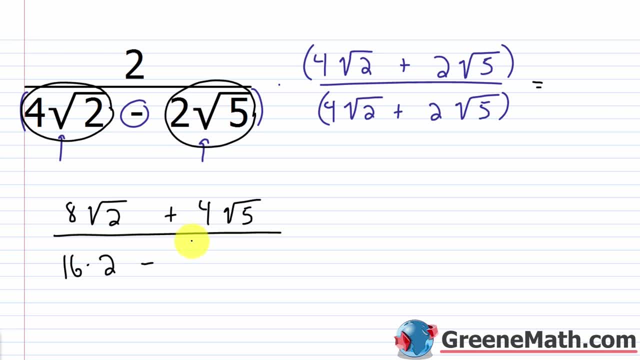 Then minus it would be this guy squared. If we square 2, we get 4.. If we square the square root of 5, we get 5.. So what we end up with is what We have: 8 times the square root of 2 plus 4 times the square root. 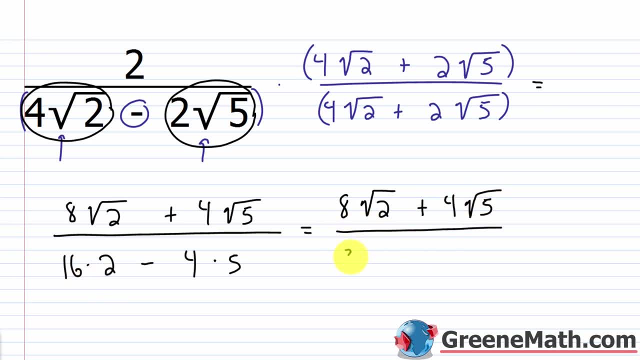 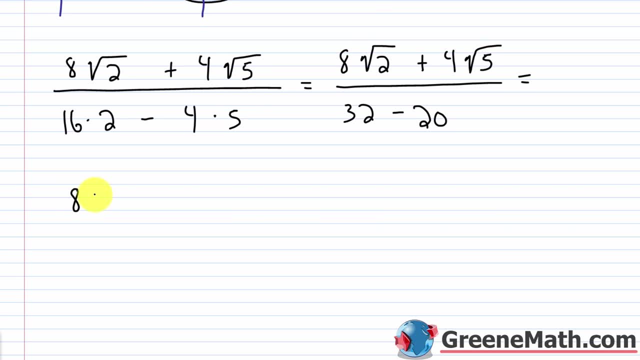 of 5 over 16 times 2 is 3.. 32 minus 4 times 5 is 20.. So we say this is equal to: we'll have 8 times the square root of 2 plus 4 times the square root. 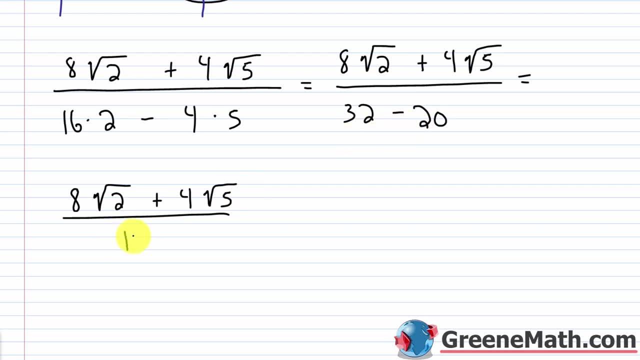 of 5 over 32 minus 20 is 12.. I could simplify a little further because I could factor a 4 out from the numerator, cancel it with a common factor of 4 in the denominator. So if we did that we'd have 4 times the quantity. 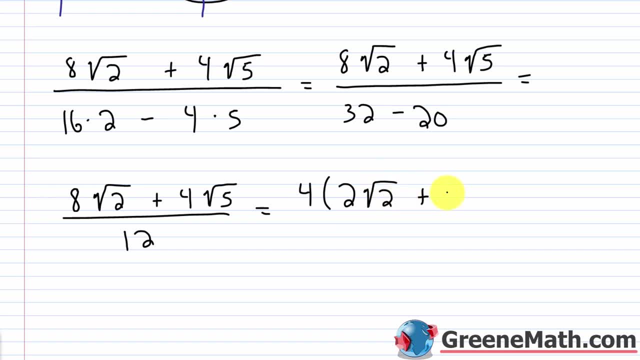 Inside of parentheses. you'd have 2 times the square root of 2, plus you'd have the square root of 5 over. you could write 12 as 4 times 3, or you could just keep it as 12, it doesn't really matter. 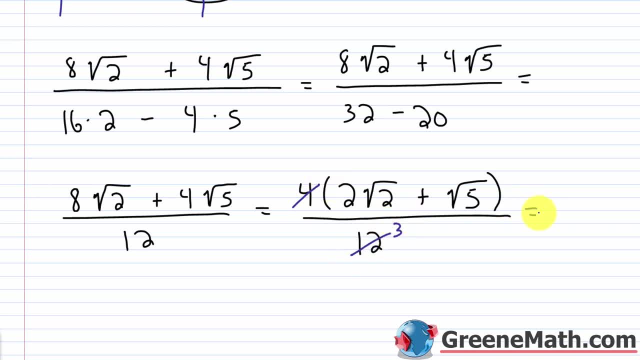 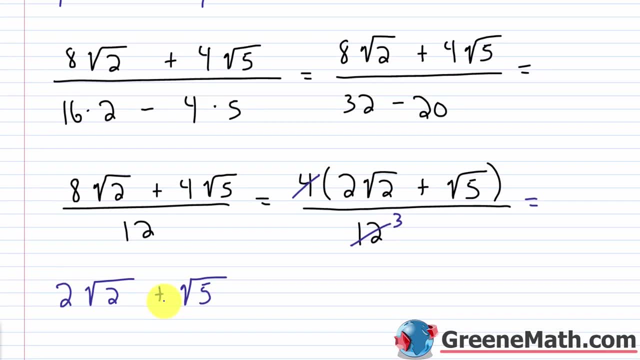 You can cancel this with a factor of 4 here, so this would be 3 now, And so our final answer would be 2 times the square root of 2 plus the square root of 5, and this is over 3.. 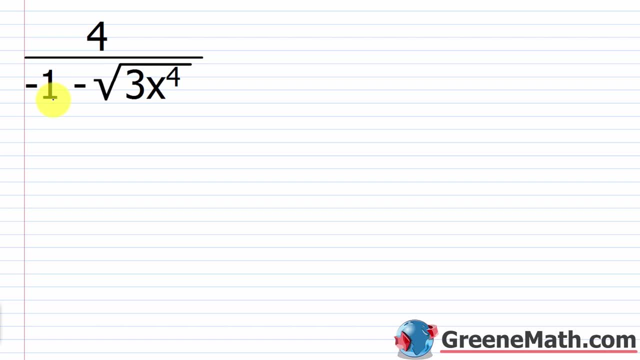 Let's take a look at another one. So we have 4 over negative 1, minus the square root of 3x to the fourth power. Now if you notice something that you can simplify like you have x to the fourth power under a square root symbol, 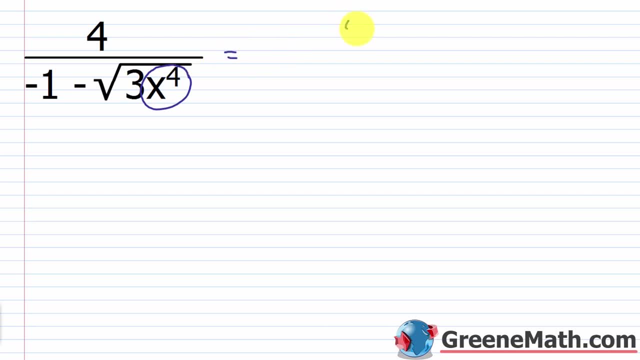 go ahead and simplify that first. So let's say this is 4 over, you have negative 1 minus. let's write this as the square root of 3 times the square root of x to the fourth power. So you should all know at this point that again. 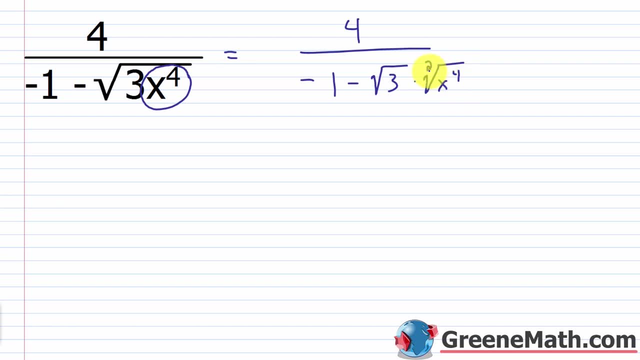 if the index is 2 and the exponent in here is a 4, you just divide. 4 divided by 2 is 2.. In other words, root of x to the fourth power is x squared, because x squared squared would give you x to the fourth. 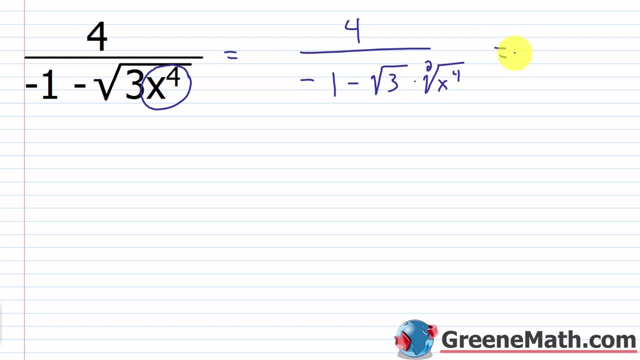 power. So we can rewrite this and say we have 4 over negative 1 minus. this would end up being again x squared. So we'll put x squared out in front times, the square root of 3.. So again I have two terms for my denominator and all I want to do is multiply the numerator and denominator. 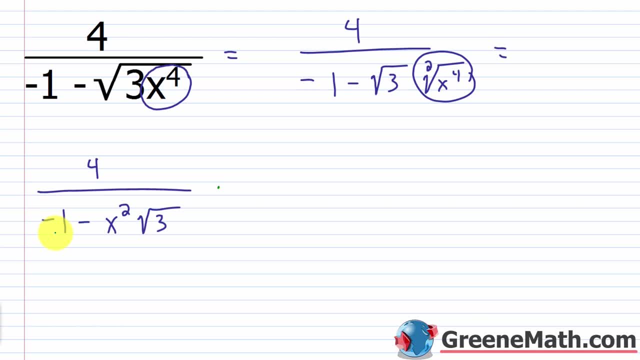 by the conjugate of this denominator. So negative 1 will stay the same and x squared times the square root of 3 will stay the same. We just need to change the sign. If this is a minus, it will become a plus Negative 1 plus x squared times square root of 3.. All right, so let's put this: 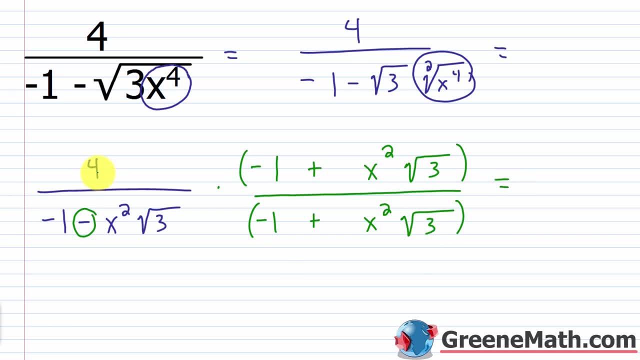 inside of parentheses. and let's see what happens: 4 times negative 1 is negative 4. then 4 times negative 1 is negative 4.. So I'm going to multiply the denominator by the conjugate of times x squared times square root of 3 would just be plus 4x squared times square root of 3.. 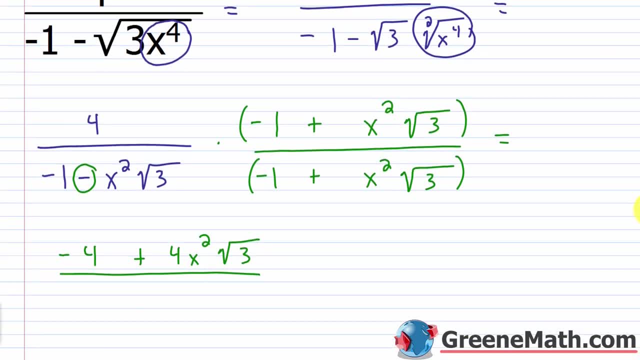 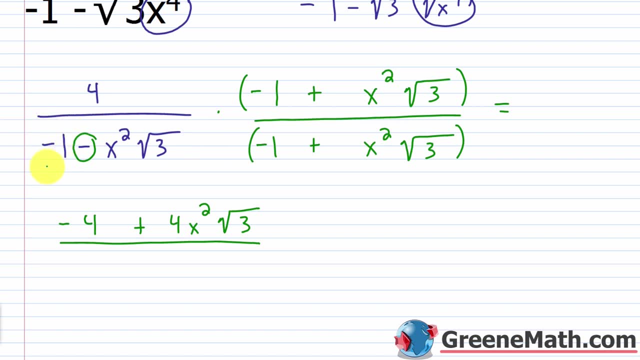 Then this is over, For in the denominator. here again we could skip through using FOIL and just use our shortcut. We know we would just square the first one. So if I squared negative 1, we would get 1.. Then we'd have minus. We would square this guy right here: x squared, squared. 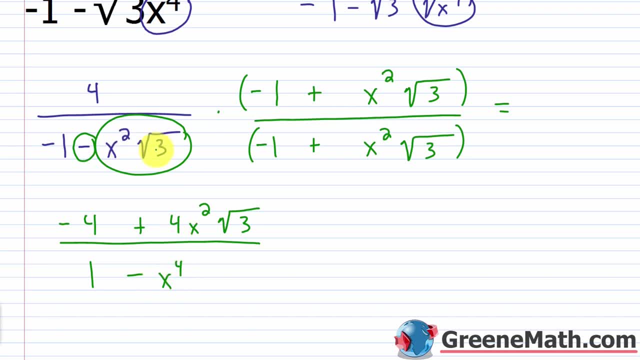 is x to the fourth power, And then the square root of 3 squared is 3 times 3.. So what is this going to be equal to? We'll have negative 4 plus 4x squared times the square root of 3. 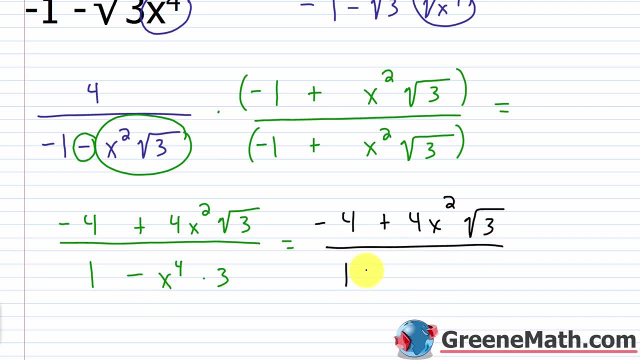 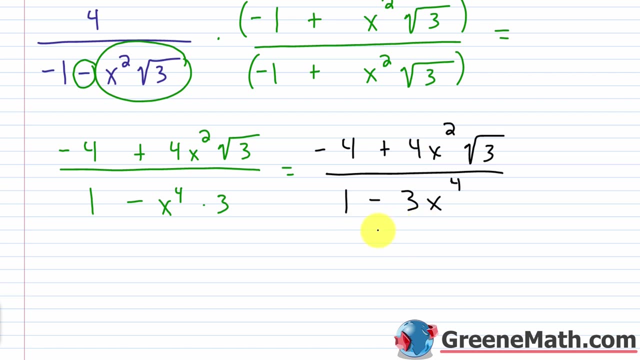 over, We would have 1 minus and you can just write this as 3x to the fourth power. Now is there anything else I can do to simplify here? Well, I could factor out a 4 or a negative 4 from the numerator, but nothing I can really cancel that with in the denominator. There's not. 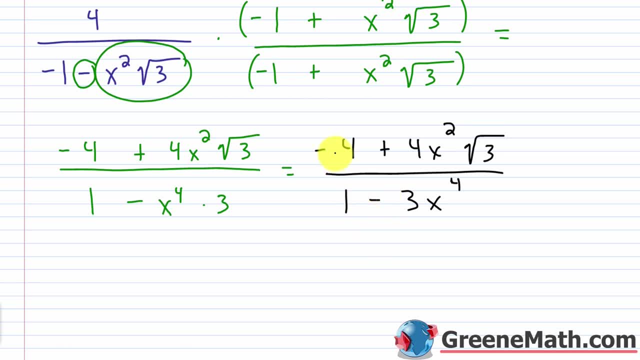 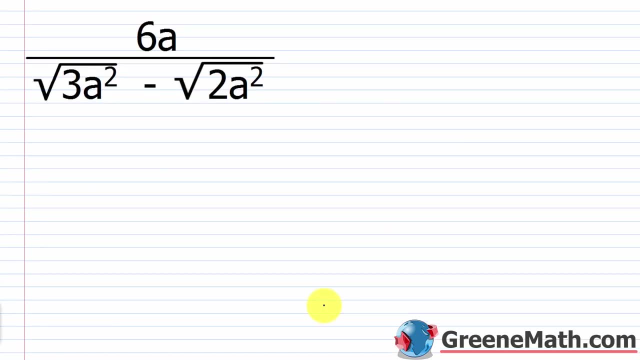 really anything else we can do to simplify. So we just report our answer as negative. 4 plus 4x squared times the square root of 3 over 1 minus 3x to the fourth power. All right, let's take a look at another one. So suppose we see 6a over. you have the square root of 3x squared minus the. 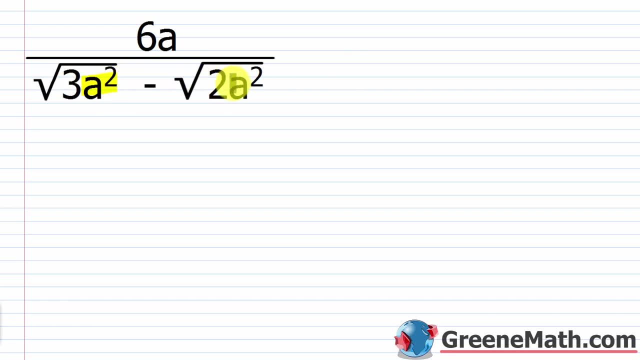 square root of 2a squared Again. if you see stuff you can simplify, go ahead and do so. So we would have 6a over. If I just write this as 3x to the fourth power, we would have 6a over. So if I just 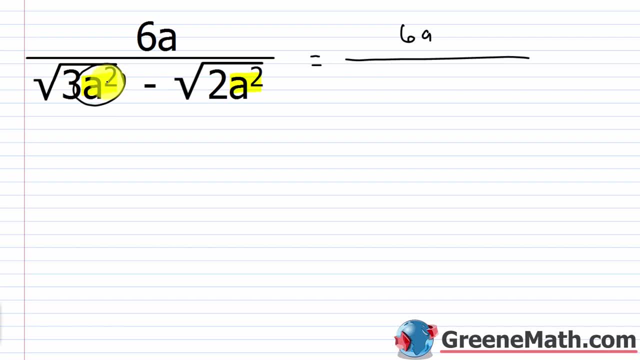 pull this out. remember, the square root of a squared is just a, So we would have a times the square root of 3, minus. same thing here: square root of a squared is a, So a times the square root of 2.. Now again, all I want to do is multiply the numerator and denominator by the. 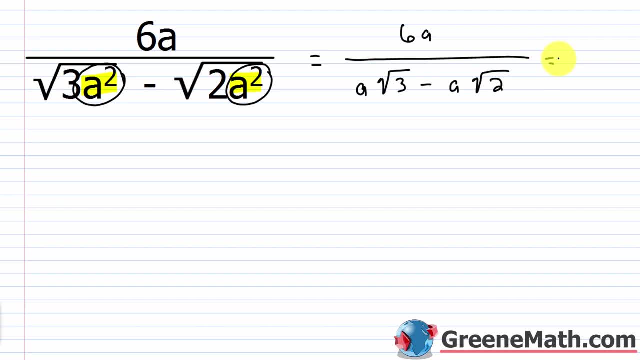 conjugate of this denominator. So let's just rewrite this real quick. We'll have 6a over. We have a times the square root of 3 minus a times the square root of 2.. So we're going to multiply this by again the 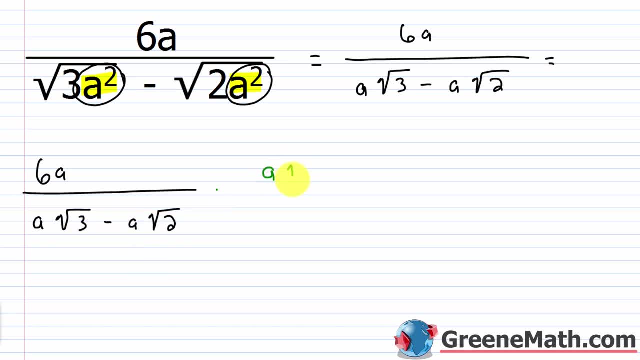 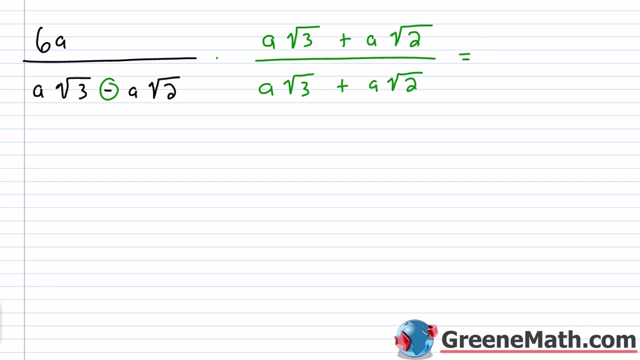 conjugate of the denominator. So we're going to have a times the square root of 3 plus right, instead of minus- a times square root of 2.. So what are we going to do? We'll have 6a times a times square root of 3.. So that would give us 6a. 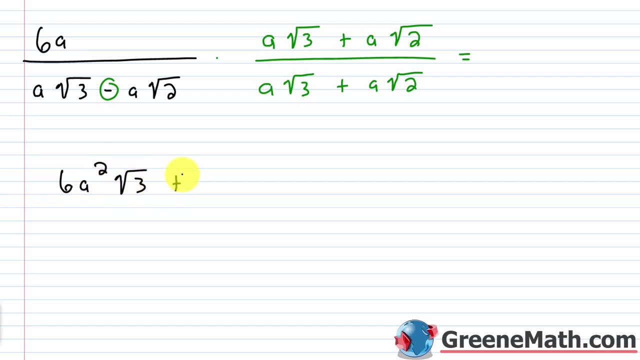 squared times square root of 3.. Then, plus 6a times a times square root of 2, would be 6a squared times square root of 2.. And then this is over Again. for these we could use our special products formula. So I'll take the first guy and square it. So I'd have a squared. 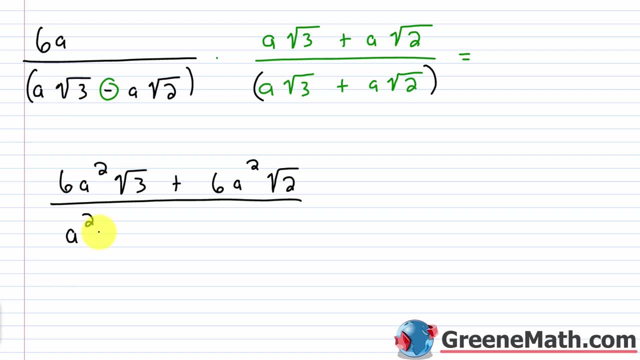 times, the square root of 3 squared is 3.. Then you'll have minus. We take this guy and square it, We'll have a squared. Now there is something I can cancel In every term of the numerator and in every term of the. 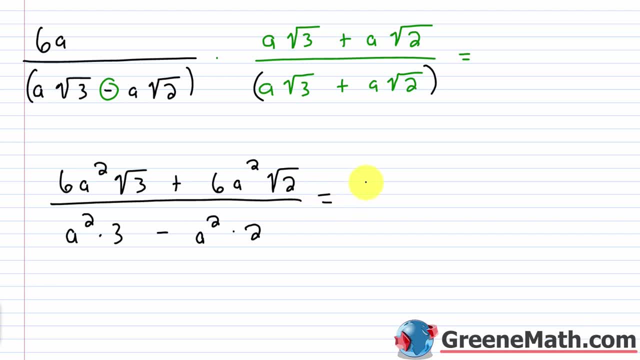 denominator. you have an a squared So you can go ahead and factor that out. So if we factor out an a squared, we'd be left with 6 times square root of 3 plus 6 times square root of 2 over down here. if we factor out an a squared, 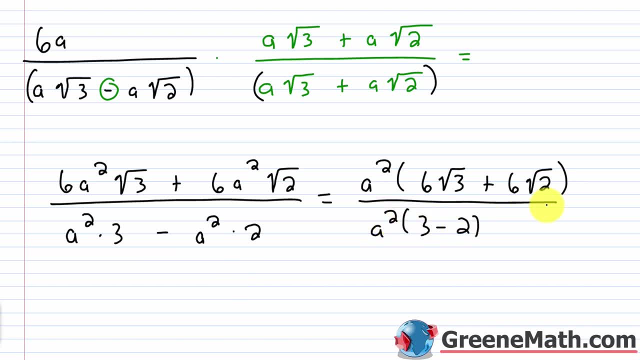 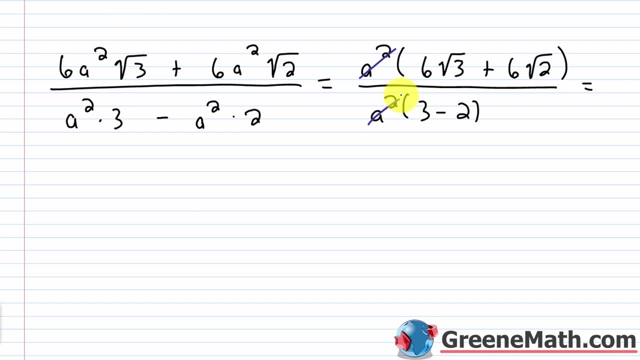 we'll be left with 6 times square root of 2.. with 3 minus 2.. So what does that give us? This is going to cancel with this, And so what we're going to end up with is 6 times the square root of 3 plus 6 times the square root of 2.. Now this: 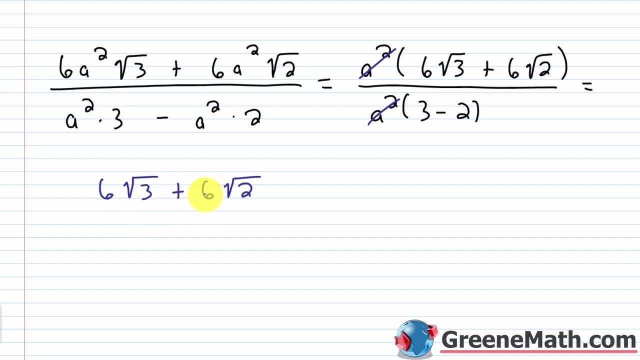 is over 3 minus 2, which is 1.. Now I could put it's over 1, or I could just leave it like it is, because anything over 1 is just itself. So our answer is just 6 times the square root of 3 plus. 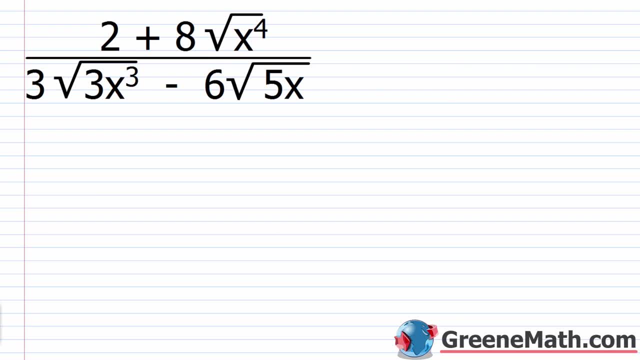 6 times the square root of 2.. All right, again, let's take a look at another one. So we have 2 plus 8 times the square root of x to the fourth power, over 3 times the square root of 3x cubed. 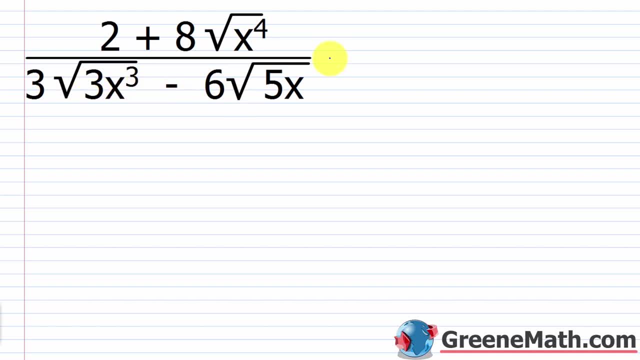 minus 6 times the square root of 5x. So again, if there's something you could simplify, go ahead and do that before you start. So we could simplify this, We could simplify this, And that looks like that's it. So we'd have 2 plus 8 times what The square root of x to the fourth power is x squared. 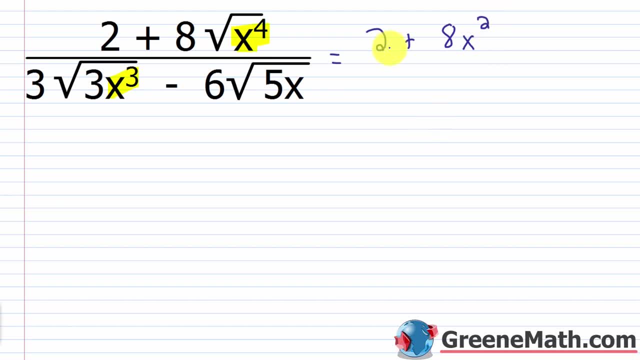 So 8x squared And if you wanted to, you could reorder that and say you have 8x squared plus 2.. Doesn't really matter, Then this is over For this guy right here. if we have the square root of x cubed, we could say that we had the square root of x squared times the square root. 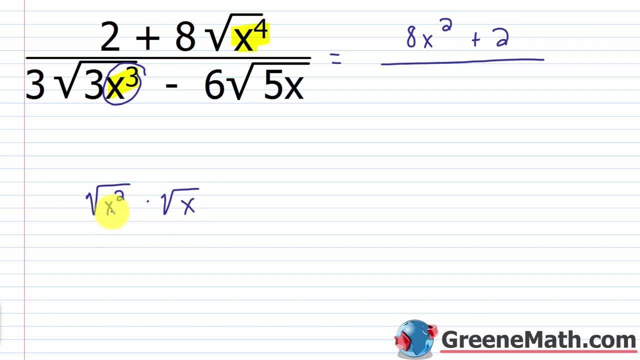 of x. All right, we can break that up. The square root of x squared is x. So what? we can write this as 3x times: you'll have this guy, and you'll have this guy, And you'll have this guy and you'll have. 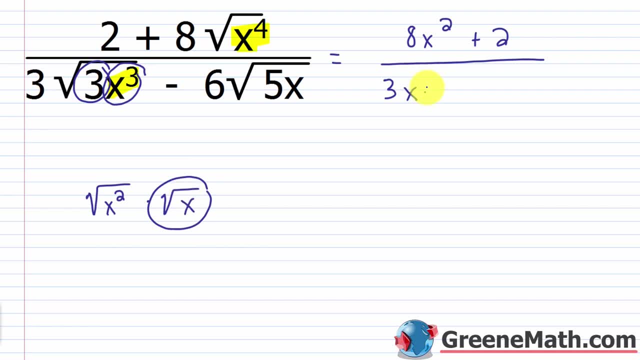 this guy. So the square root of 3 times the square root of x. we'll just write that as the square root of 3x and then minus 6 times the square root of 5x. Now again, once we've got to, 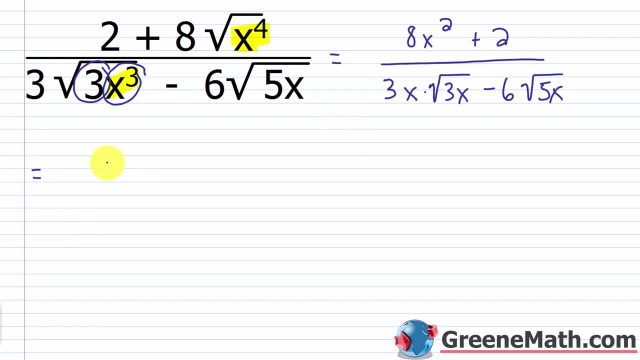 this step. all we want to do is multiply the numerator and denominator by the conjugate of this denominator. So we have 3x times square root of 3x minus 6 times the square root of 5x. We're going to multiply that by the square root of 3x. So we're going to multiply that by the. 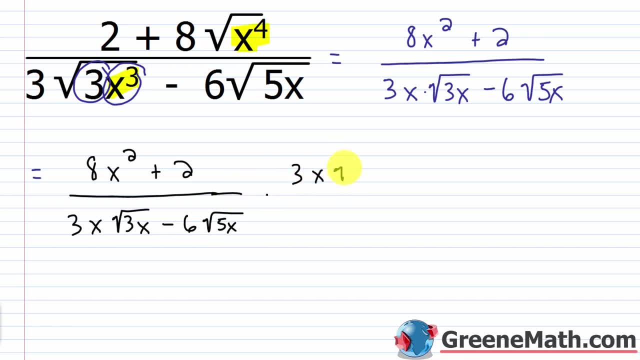 square root of 3x, We'll have 3x times the square root of 3x. Instead of this being minus, we'll put a plus And then 6 times the square root of 5x. This is over, Again, 3x times the. 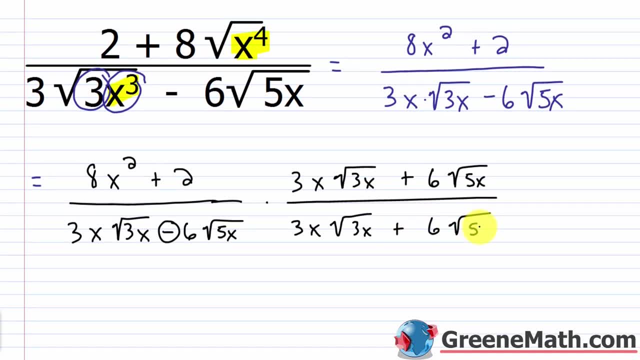 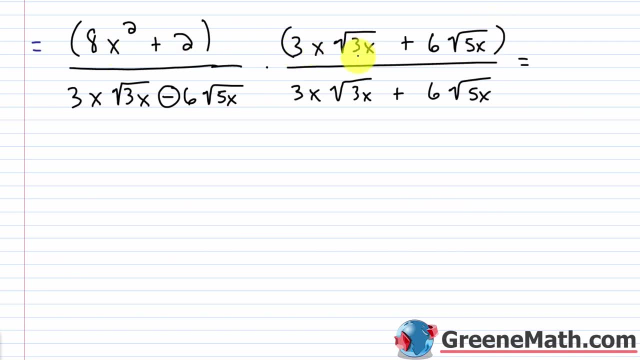 square root of 3x plus 6 times the square root of 5x. We're going to use FOIL in our numerator, So 8x squared times 3x times the square root of 3x, You would do 8 times 3, that's 24.. 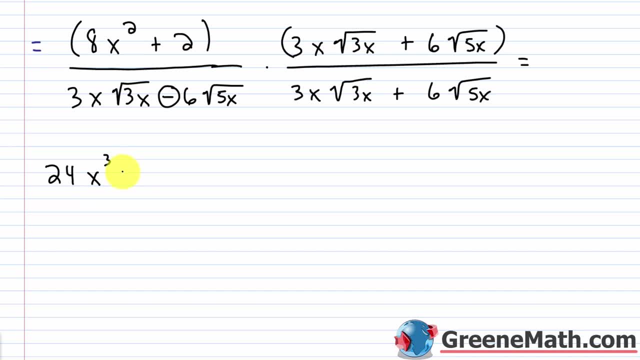 You would do x squared times x, that's x cubed, And then times the square root of 3x. For the outer, you would have 8x squared times 6 times square root of 5x. 8 times 6 is 48, so plus 48. And then you'd have x squared and then times the. 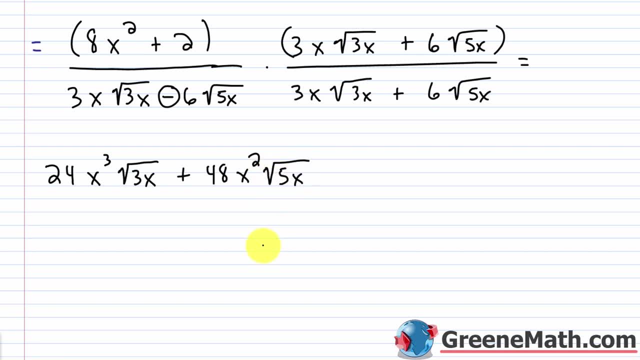 square root of 5x. For the inner we have 2 times 3x times the square root of 3x, So plus 6x times the square root of 3x. And then, for the last, we have 2 times 6 times the square root of 5x, That's plus 12 times the. 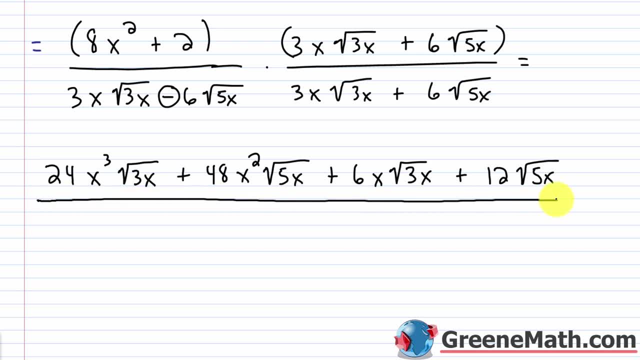 square root of 5x. All right, so then this is over In the denominator. again, I'm going to use my special products formula: 3x times the square root of 3x squared. So 3x squared would: 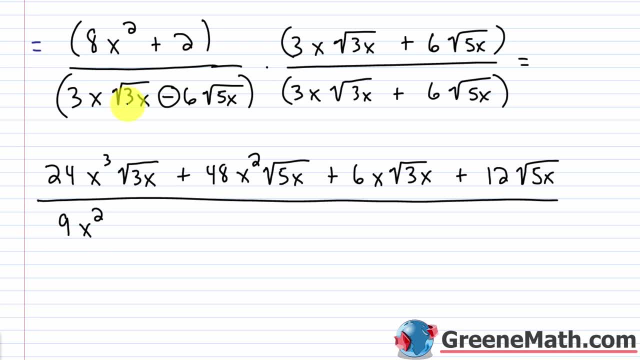 be 9x squared. The square root of 3x squared would just be 3x. So times 3x, And if we do this calculation now, we'd have 27x cubed. So let's just go ahead and write that. 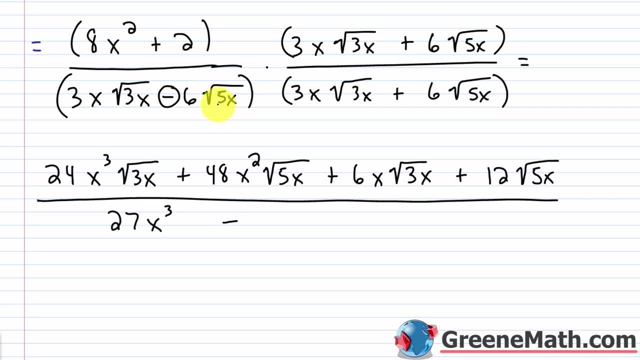 Then minus From the second guy: squared 6, squared is 36.. And then the square root of 5x squared would just be 5x. So 36 times 5 is 180.. So we'll put minus 180 and then times x. 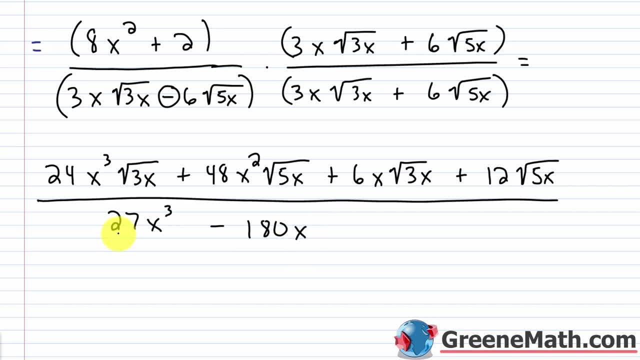 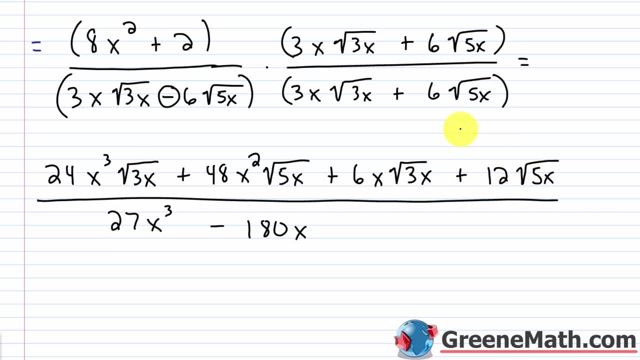 that from right here And when we talk about in terms of being able to factor out an x and cancel. So that's not going to work. But everything is divisible by 3.. So we could pull out a 3 from the numerator and from the denominator. So that would leave me with 8x cubed times the 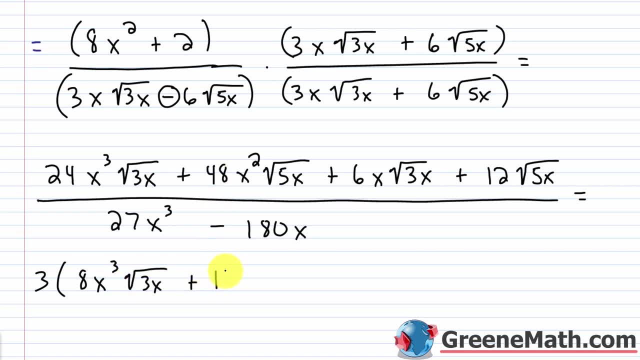 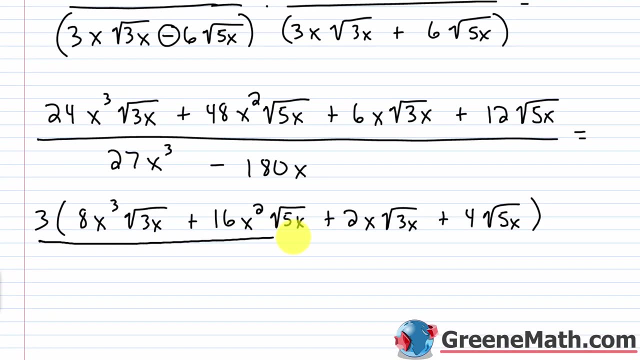 square root of 3x plus 16x, squared times the square root of 5x plus 2x times the square root of 3x Plus 4 times the square root of 5x. Then this is all over. If I pulled out a 3, I'd have 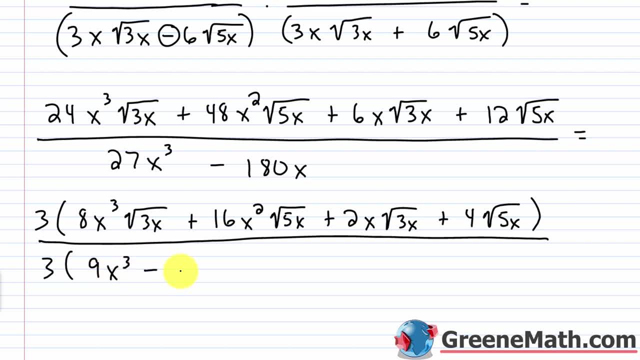 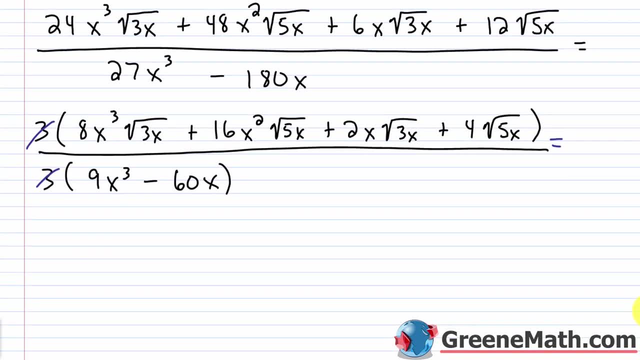 3 times, You'd have 9x cubed minus 60x. So let's go ahead and cancel this 3 with this 3.. And what are we going to be left with? We're going to have 8x cubed times the square. 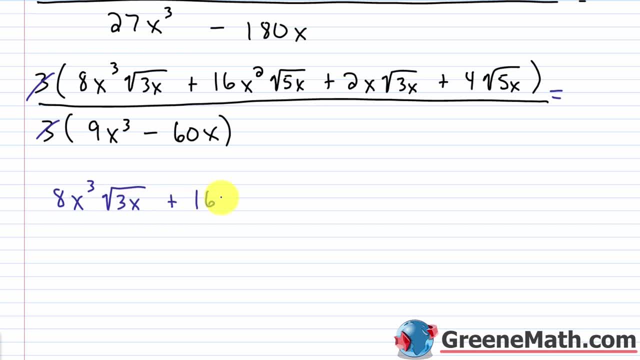 root of 3x plus 16x squared times the square root of 5x, plus 2x times the square root of 3x, plus 4 times the square root of 5x, And this is all over. You'll have 9x cubed minus 60x. 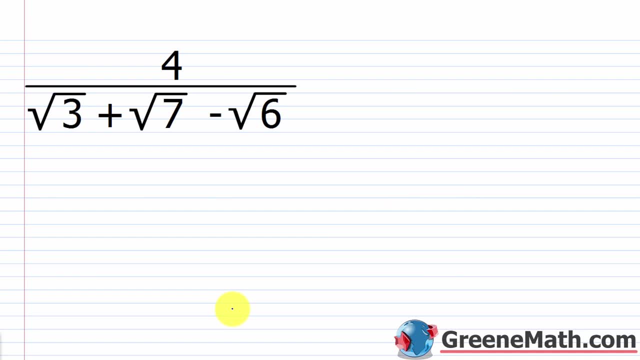 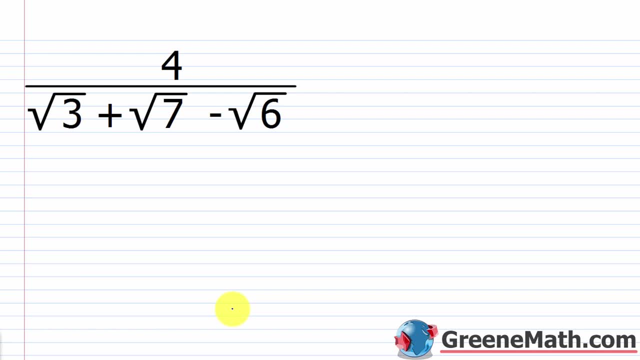 on this because it's a very popular bonus question for a homework or for even a test. So let's say, you saw something like 4 over the square root of 3, plus the square root of 7, minus the square root of 6.. You don't have two terms in this denominator, You have three. So how do we? 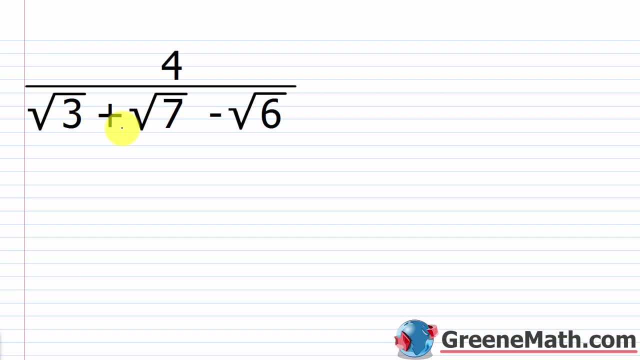 rationalize here. Well, we're going to use the same concept, but what we're going to do is we're going to group two of the numbers together. So let's say we grouped the first two numbers together. Let's just say we're going to group the first two numbers together. So let's just say we'm going to 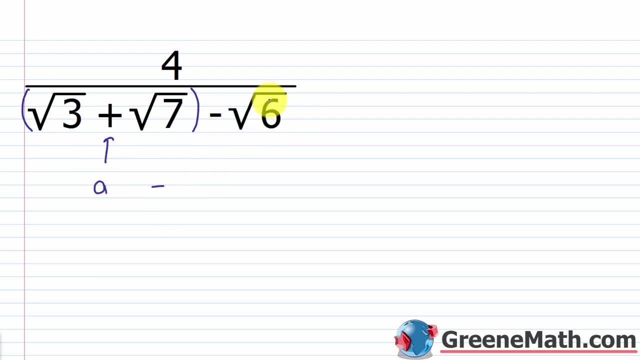 we call this a, then we have minus, and then let's just call this one b, so we have a minus b. if i had two terms in the denominator, and one was a and one was b, and i had this minus sign here, the conjugate of that would be a plus b. so again, with this being a, this square root of three plus the square root. 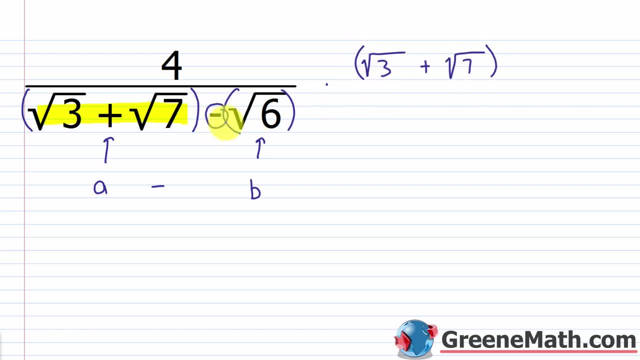 of seven. i would just change the sign here. this is minus, so now it's going to be plus, and then my b is the square root of six. then this is over again. you do the same thing. so square root of three plus square root of seven plus square root of six. okay, so let's do our multiplication. we're going to see. 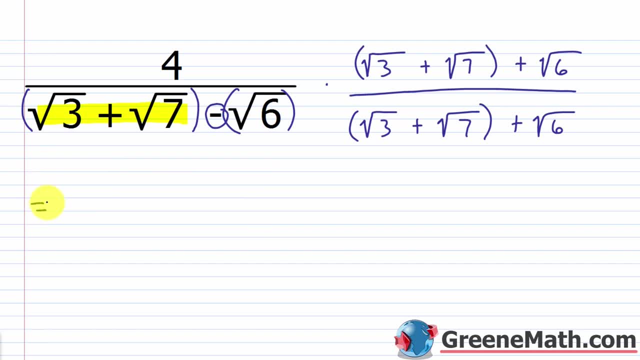 where we're at. so four times the square root of three would be four times square root of three. then plus four times square root of seven is just four times square root of seven. then plus four times square root of six is four times square root of six. 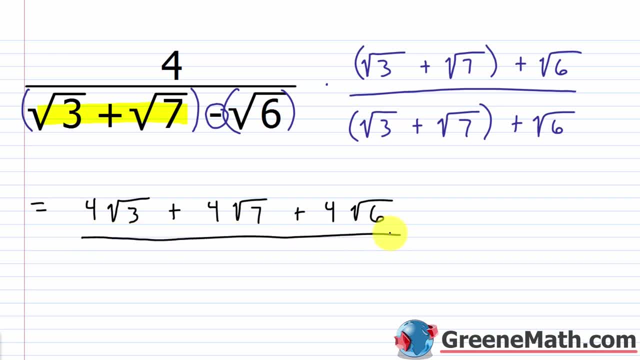 then this is all over. now you can go through this the long way and you could take, let's say, the square root of three multiplied by every term here. then you could take square root of seven multiplied by every term here. you could take negative square root of six multiplied by every. 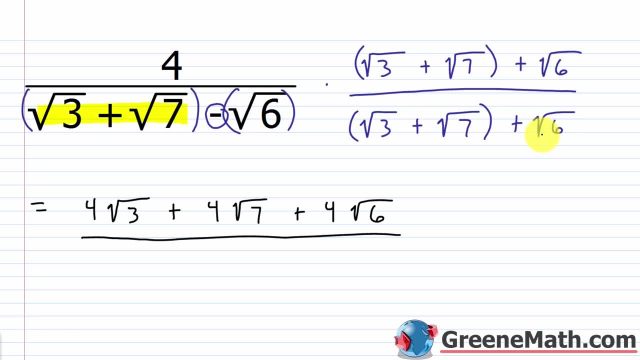 term here, and then you can cancel all those things. or again you can realize the shortcut. i can take this and multiply it by this. so in other words, i could take this first part, or we labeled as a, and i could square it, so i could have the square root of three plus the square root of seven squared, then i could subtract away. 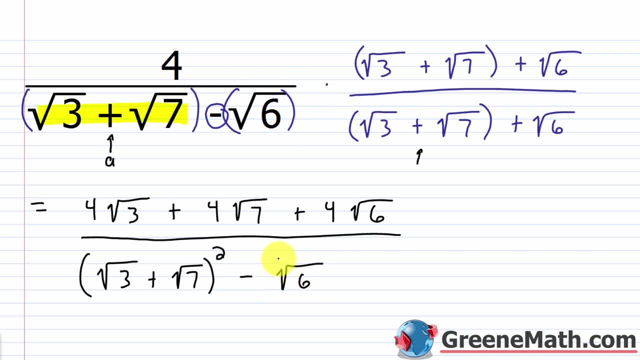 this second guy, which is the square root of six squared, i could treat it again just like this was a and this was b. so if i had a minus b times a plus b again, that's what i would do. all right, that's my special products for you, all right? so i'm going to do that again. so i'm going to do this. 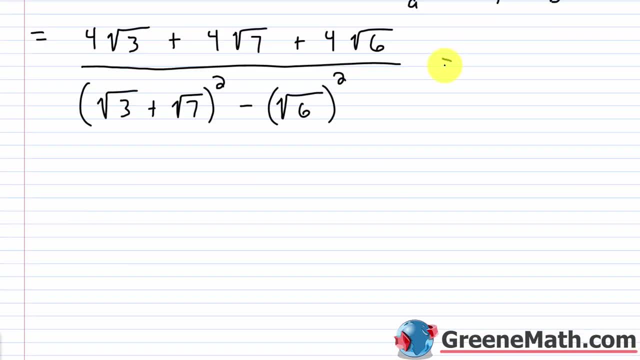 formula, no different here. all right, so let's simplify here. so we have four times the square root of three, plus four times the square root of seven, plus four times the square root of six. this is over. we can use the special products formula for this as well. i would have the first. 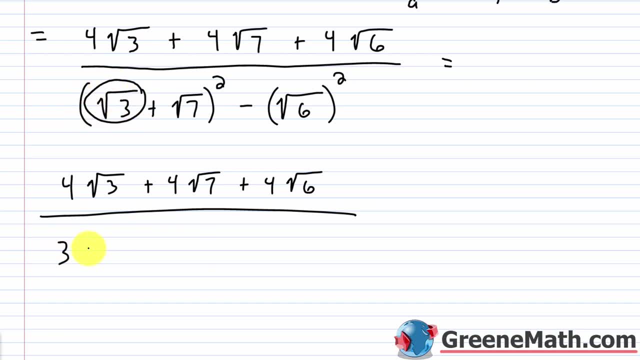 guy squared. so the square root of three squared is three plus two times the first guy times the second guy, so two times the square root of three times the square root of seven would be two times the square root of three times the second guy, so two times the square root of three times the. 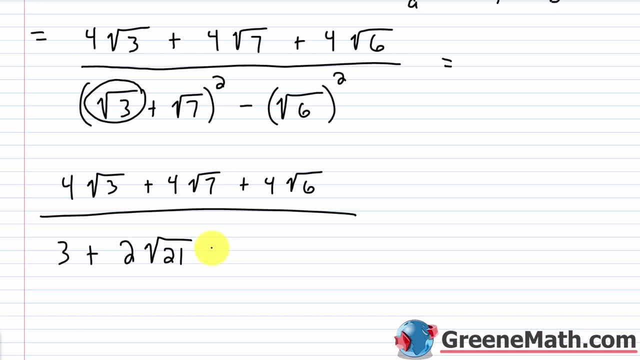 square root of twenty one, and then you would have plus the last guy squared, so the square root of seven. squared is seven. now three plus seven is ten. so you might as well just put this as ten plus two times the square root of twenty one, then minus. lastly you have the square root of six. 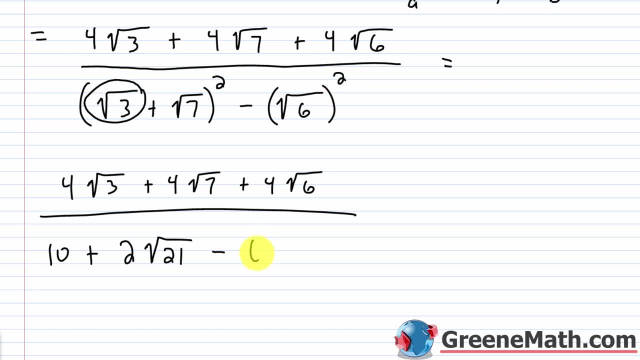 squared. so if i square the square root of six, i get six. so ten minus six is four. so this is four plus this guy. now you might say: hey, that didn't work, we still have a radical in the denominator. yeah, we do, but what is this? this is a binomial. 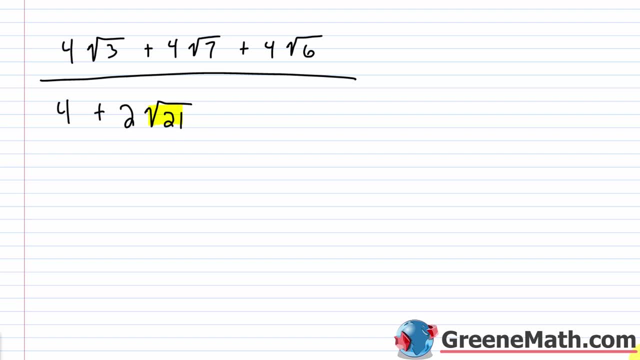 denominator. we already know how to do that, so we took an extra step and now we're at a point where we can just multiply again by the conjugate four minus two times square root of twenty one, over four minus two times square root of twenty one. and again, i know this is a very tedious problem, but 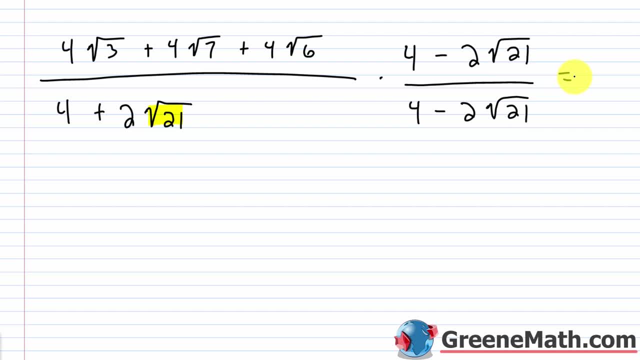 it's something that, again, if you get this as a bonus on a test, it's really worthwhile to know how to do something like this. so what we're going to do is we're going to take four times square root of three and multiply it by four, so that's going to give us. 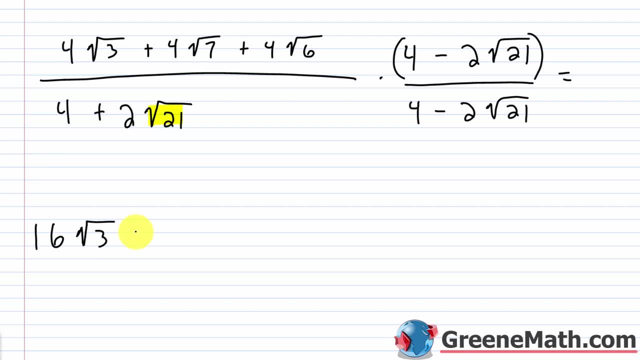 sixteen times the square root of three. then we'll take four times square root of three and multiply it by a negative two times square root of twenty one. four times two is eight. square root of three times square root of twenty one is going to be the square root of sixty three. then next you'll. 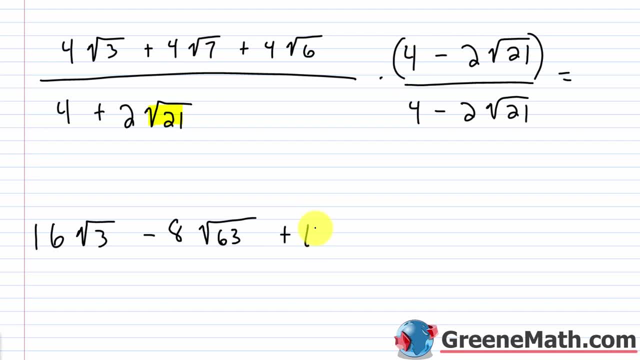 have plus, you have four times square root of seven times four, that's sixteen times square root of seven. then next we have four times square root of seven, times negative two times square root of twenty one. that'll be negative eight times the square root of one hundred forty seven. 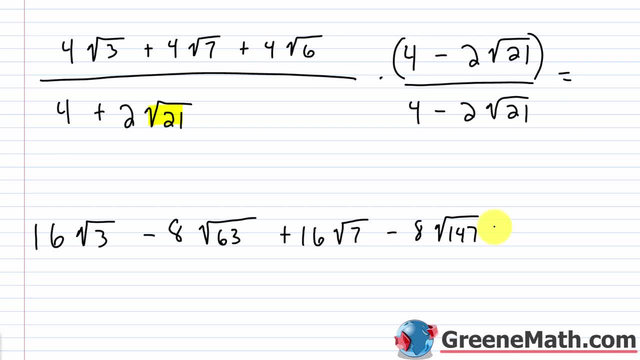 then we have plus four times square root of six times four, that would be sixteen times square root of six. and lastly- let me kind of rewrite this so i can fit it all on the screen- so we have sixteen times square root of three, minus eight times square root of sixty three. 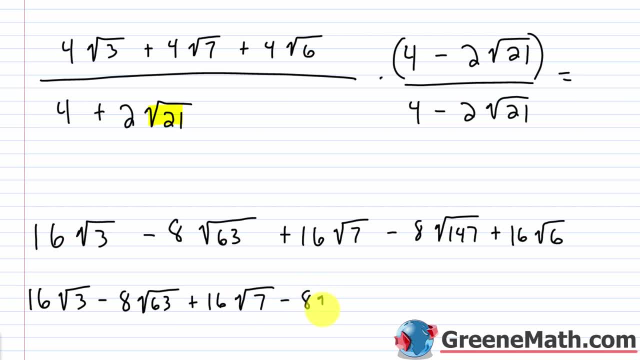 plus sixteen times square root of seven minus eight times square root of one hundred forty seven plus sixteen times square root of six. just erase this and we'll kind of drag this up, okay, so the last one was four times square root of six, times negative, two times square root of twenty one. 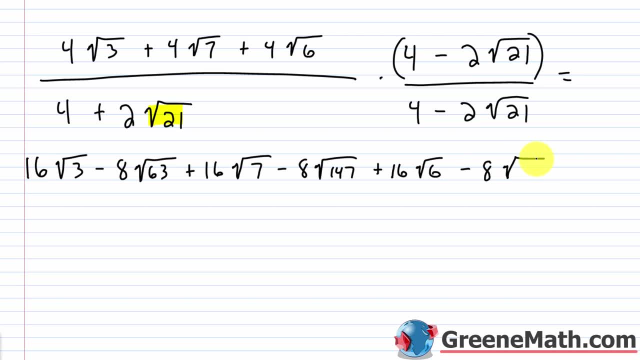 so that's negative. eight times the square root of one hundred twenty six. okay, now this is all over again. if i'm multiplying here and i have conjugates, i just need to do the four times square root of twenty one. first guy squared, So 4 squared is 16 minus the last guy squared, 2 squared is 4.. Square root of: 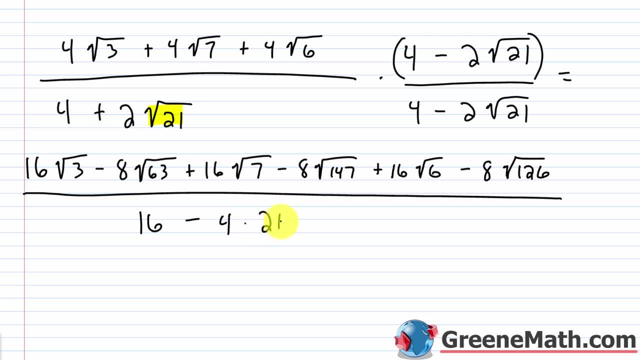 21 squared is 21.. So what's 4 times 21?? That's going to give us 84.. So 16 minus 84. And if we do 16 minus 84, we'll get negative 68. So let's write negative 68 here. You notice that the 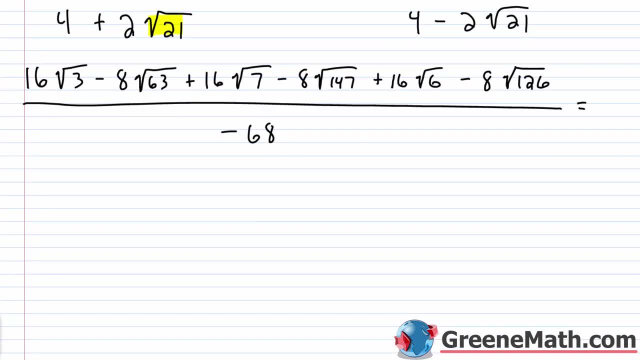 numbers that are multiplying. these radicals are all even numbers. You've got 16,. you've got a negative 8, 16,, a negative 8, 16, and a negative 8.. Now this is negative 68.. So if we think about, 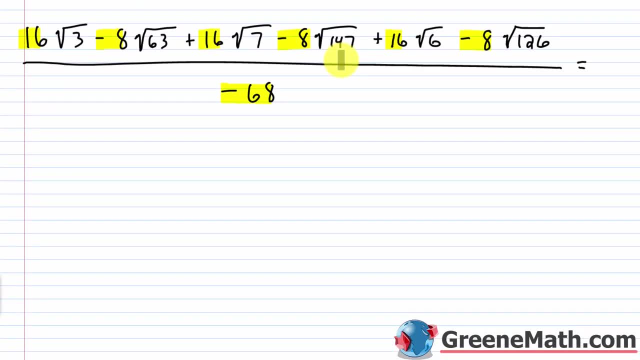 between numerator and denominator there would be a common factor of 4, or you could also do negative 4.. It depends on what you want to do. I'd prefer to cancel a common factor of negative 4.. I just like to report my denominator as positive, So in the numerator, instead of 16, I'll have 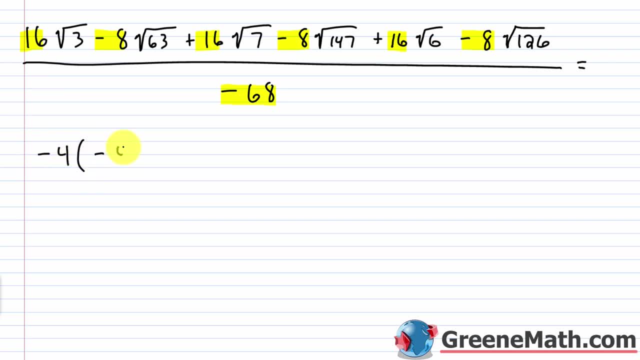 negative 4.. So we'll put negative 4 on front times, negative 4 times square root of 3.. And then we'll put negative 4 on front times, negative 4 times square root of 3.. And then this would become positive 2.. So plus 2 times square root of 63.. This would become 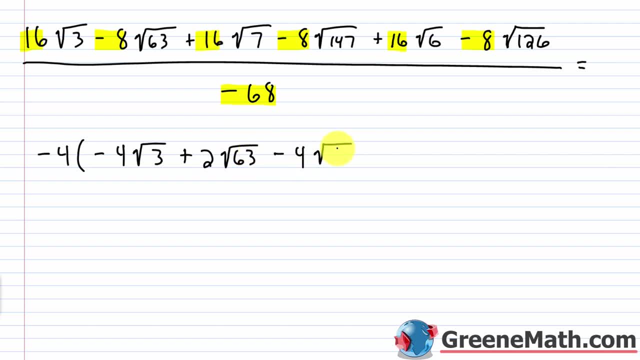 negative 4.. So minus 4 times square root of 7.. This would become positive 2.. So plus 2 times square root of 147.. This would become negative 4.. So minus 4 times square root of 6.. And lastly, 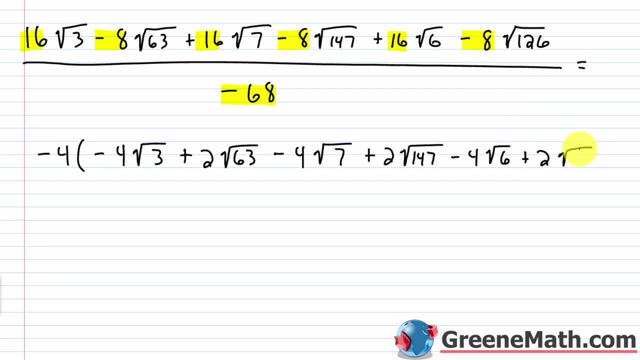 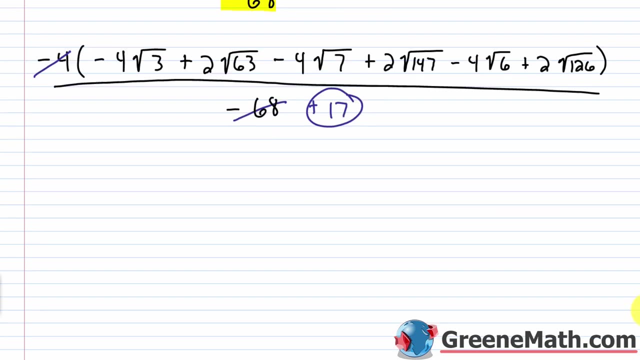 this would become positive 2.. So plus 2 times square root of 126.. Then this is all over negative 68.. Now if we cancel a common factor of negative 4 between numerator and denominator, this will end up being positive 17 down here. Now we're still not done, because there's more. 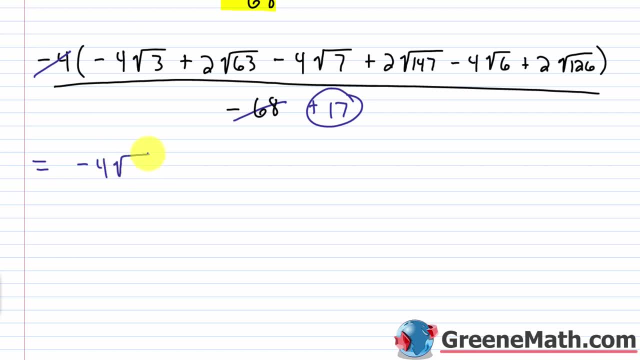 things that we can do. So I have negative 4 times the square root of 3, plus 2 times the square root of 63 is the square root of 9 times the square root of 7.. We know the square root of 9 is 3.. 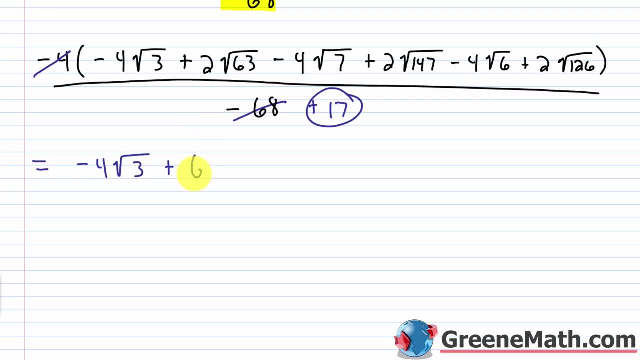 So you'd have 2 times 3,, which is 6 times the square root of 7.. Then you have minus 4 times the square root of 7.. Then you have plus 2 times the square root of 147.. Now let's stop for a second 147,. 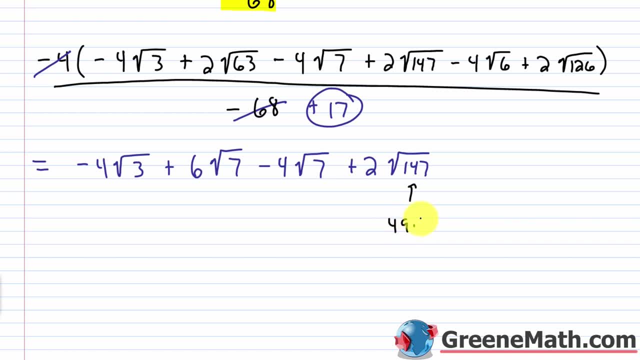 we don't work with that very often, But this is 49 times 3.. Now we know that 49 is what It's 7 times 7.. So I could say we have the square root of 49, which is 7 times the square root of 3.. 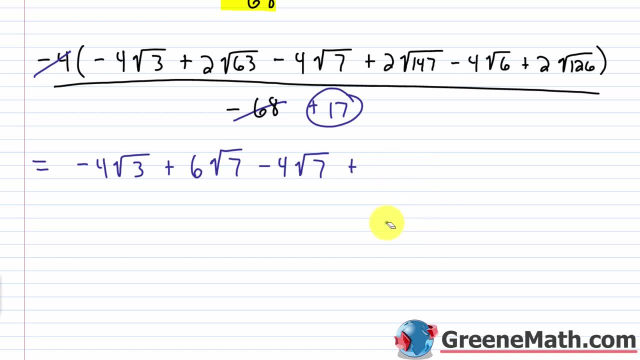 So 7 times 2 would be 14.. So this would be 14 times the square root of 3.. Then you have minus 4 times the square root of 3.. Then, lastly, plus 2 times the square root of 126.. 126 is 2 times 7, times 3, times 3 or times 9.. 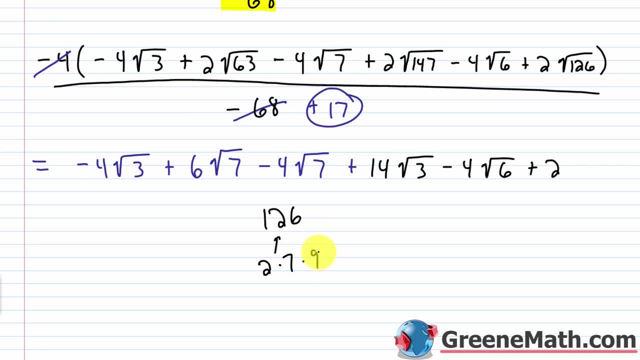 So 9 is a perfect square. So again, if we pull that out, the square root of 9 is 3.. So I could make this 2 times 3 or 6 times the square root of 14.. Okay, now, this is all over 17.. 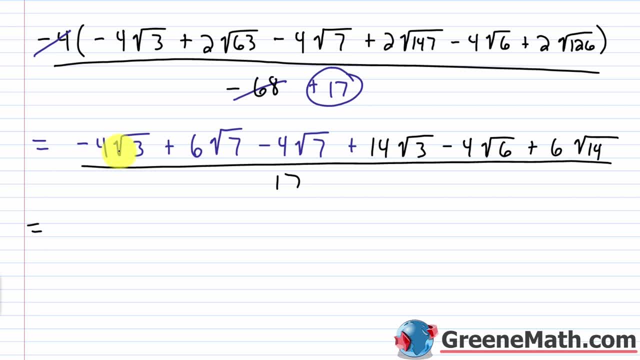 All right. so what do we have here that we can combine? You've got a negative 4 times the square root of 3 and 14 times the square root of 3.. So those are like radicals. So we can say: that's 10. 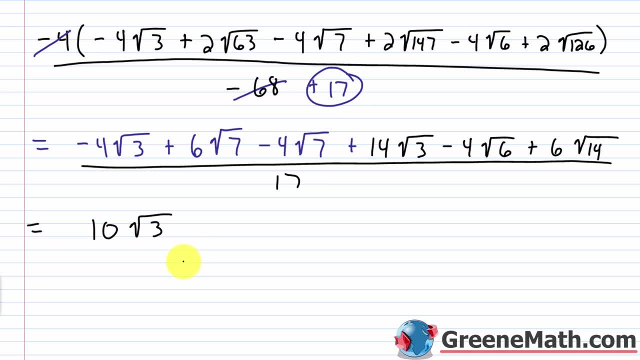 times the square root of 3.. Then we've got 6 times the square root of 7 minus 4 times the square root of 7.. Those are like radicals. We say: that's plus 2 times the square root of 7.. Then we have minus. 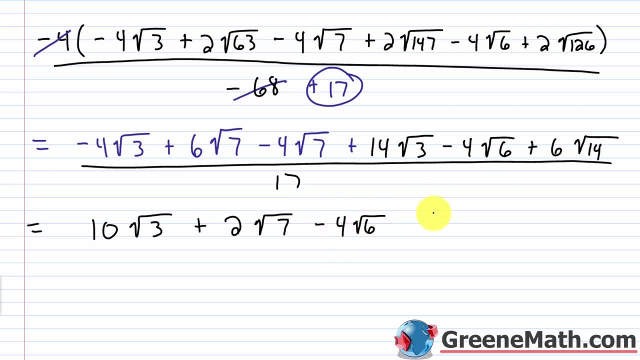 4 times the square root of 6.. Nothing we can do with that. And then, lastly, plus 6 times the square root of 14.. Nothing we can do with that. And then this is all over again: 17.. So that's going. 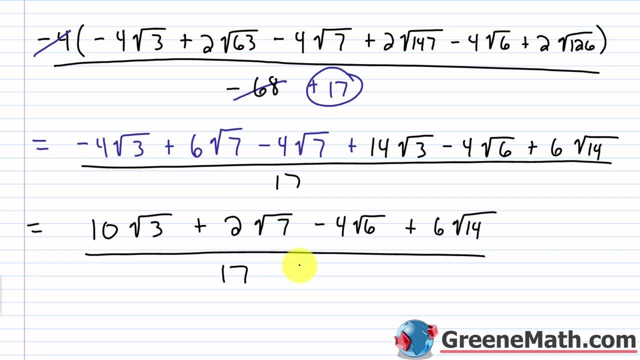 to be your final simplified answer. Nothing else we can do here And again, I know it was a long problem, I know it was very tedious, But it's something you should get used to doing, in case you get that as a bonus question on the test, Something you can do and make up for any problems. 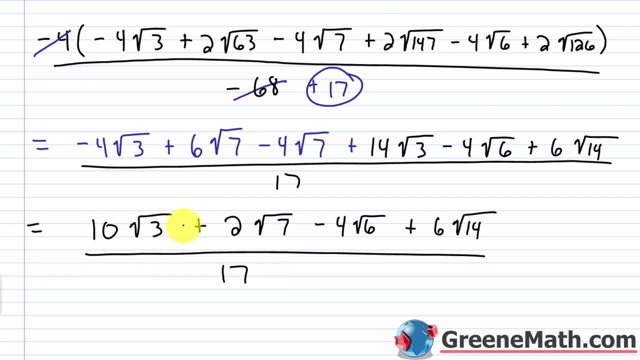 you encounter that you couldn't solve. So we've got 10 times the square root of 3 plus 2 times the square root of 7 minus 4 times the square root of 6 plus 6 times the square root of 14.. 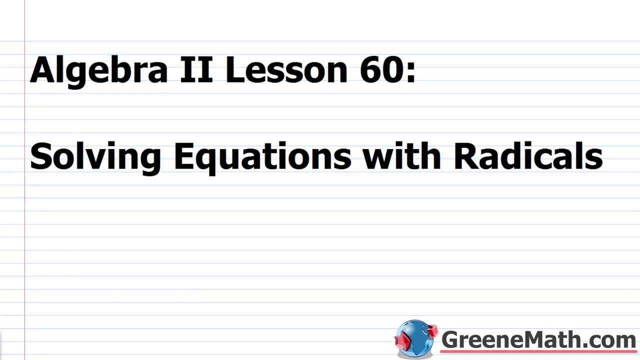 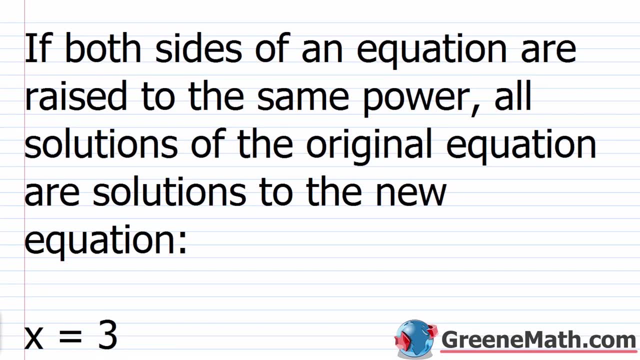 All over 17.. Hello and welcome to Algebra 2, Lesson 60. In this video, we're going to learn about solving equations with radicals. So when we start talking about solving an equation with a radical involved, we need to think about a new rule. So if both sides of an equation are raised, 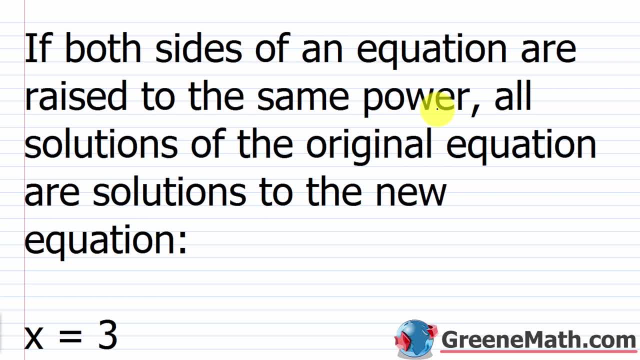 to the same power. So, just as an example, let's say I have squared both sides of an equation. All solutions of the original equation- meaning before I squared both sides- are solutions to the new equation. But the catch to this is going to be that it 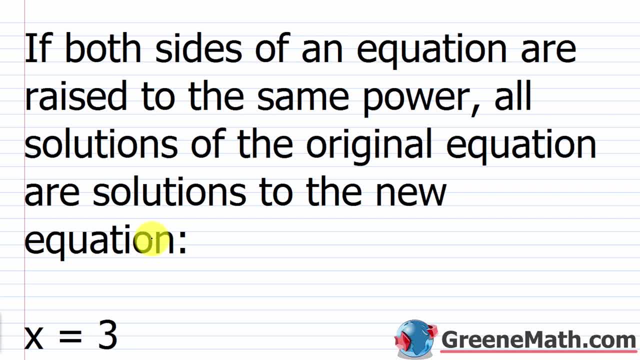 doesn't go in reverse Each solution to the new equation. in other words, once I've squared everything, if I solve that new equation, it's not necessarily going to work in the original. Okay, so we have to check for something known as extraneous solutions, And these solutions do not. 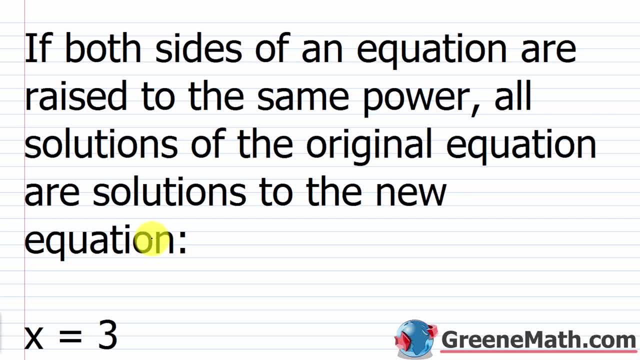 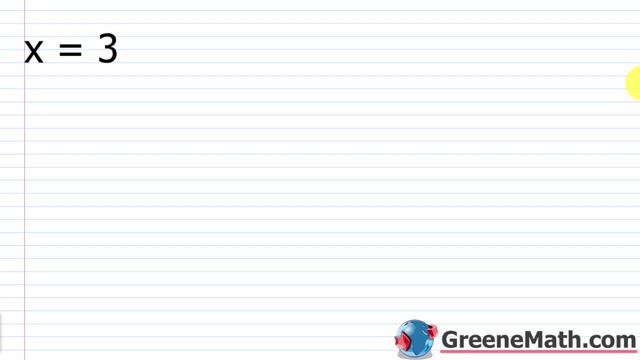 work in our original equation. So for you to understand this, here's a little simple example here, And this is very common. in any textbook you're looking at, You'll see something like x equals 3. And right now we know that if we replace x with anything, 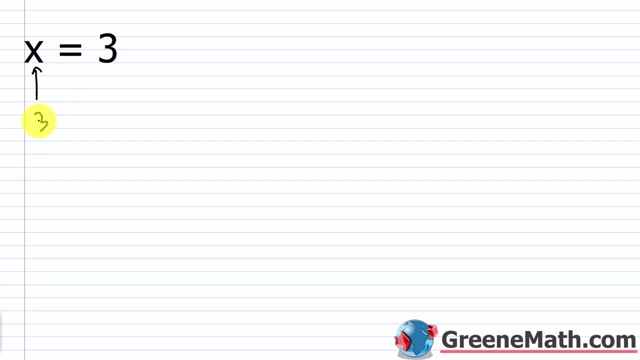 other than 3, we would get a false state. All right, I can only say that 3 could be replaced for x, So I get 3 equals 3.. All right, so now that we understand that, if we squared both sides of, 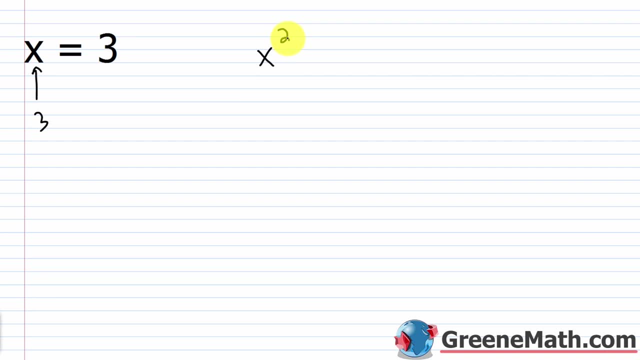 the equation, let's just say this- became x squared, And if I square 3, I would get naught. What happens? What happens here? Well, 3 is still a solution If I plug in 3. there, 3 squared equals 9.. That's. 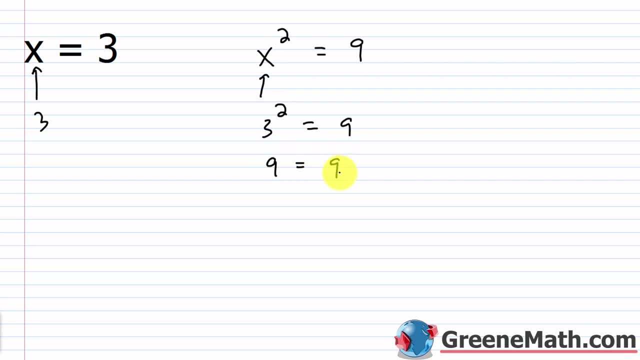 true, 9 equals 9.. So it seems like there's no problems. Everything is good to go. But remember, if I square a negative, it becomes a positive. So this is where kind of information is lost. okay, We've squared both sides and we've lost the information on whether or not it was a positive. 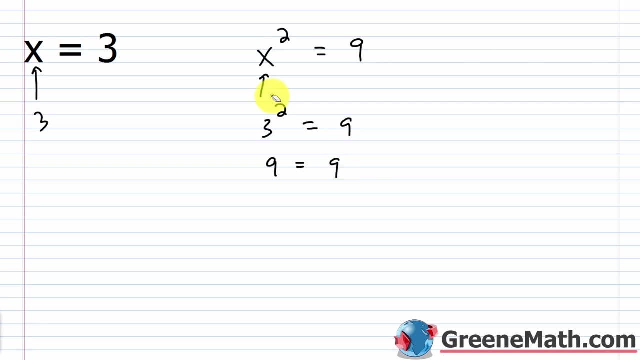 or a negative. So in other words, what I could also as a solution here is negative 3.. So if I plugged in a negative 3 there and I squared it right, the negative n to 3 would be squared. this would also be equal to positive 9.. 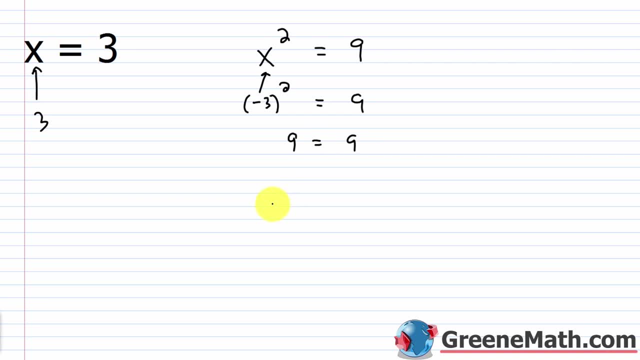 So you'd get a true statement: 9 equals 9.. So with the equation x squared equals 9, there's two solutions. Your solution set would contain negative 3 and positive 3.. But again, with the original there's only one solution: x. here can just be 3.. 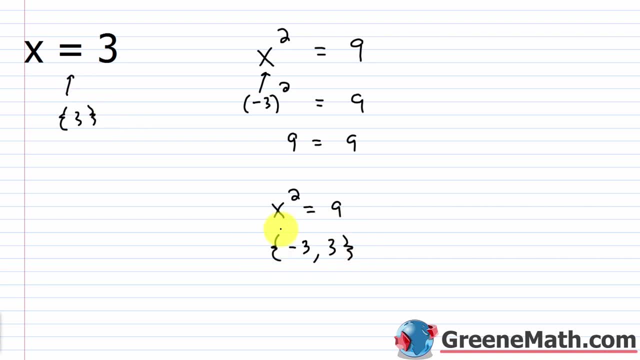 So if you've squared both sides to get to this and you end up with these two solutions, you've got to plug them back in to the original equation and you've got to figure out if they work or they don't work. You plug in a 3, you see that it works. you know that's a valid solution. 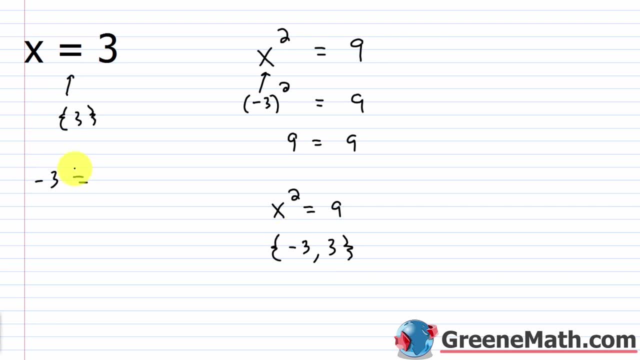 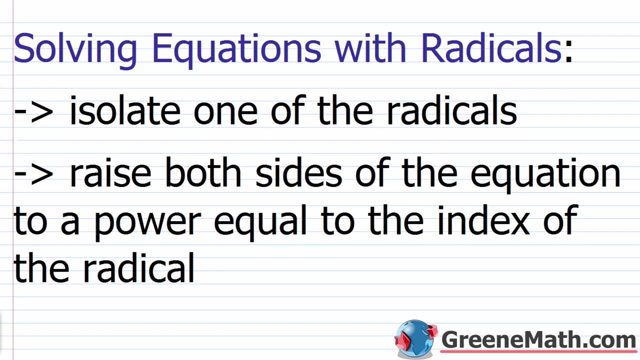 You plug in a negative 3,, you'd see that negative 3 does not equal 3.. So negative 3 is an extraneous solution. It's something you have to reject. All right, so let's look at the procedure to solve an equation with radicals. Basically, all you want to do is plug in a negative 3, and you'll. 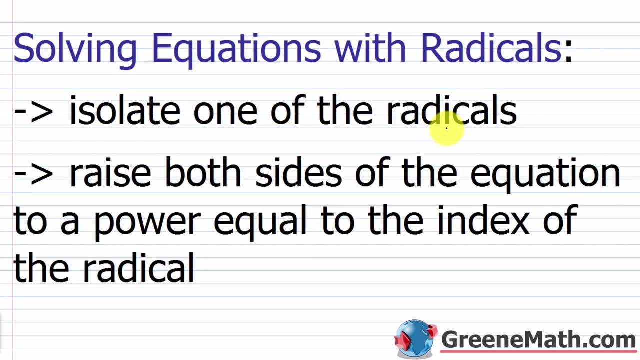 want to do is isolate one of the radicals first For your easier problems. the one you get introduced to you basically just have one radical and normally it's just a square root. So with those you just push the radical on one side you push your number or whatever else on. 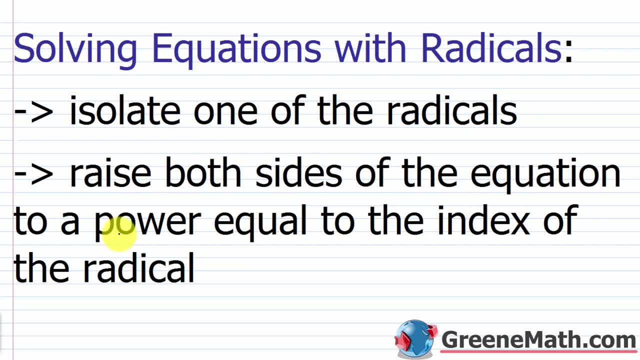 the other side, and then you're going to raise both sides of the equation to a power equal to the index of the radical. So in other words, if it's a square root, the index is a 2, so you square both sides. If it's a cube root, the index is a 3, so you cube both sides. So on. 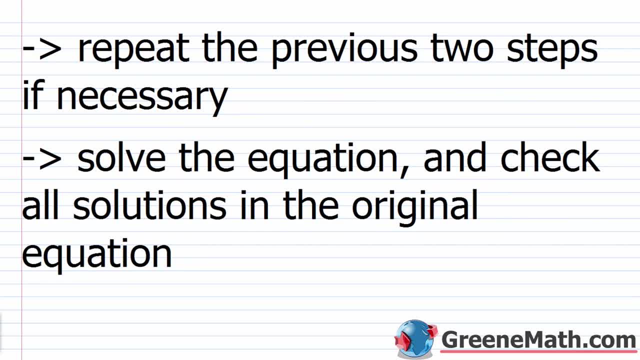 and so forth. Now with your harder problems, the ones you're going to see at the end of the section. or let's say you're doing a college algebra course, or even in this algebra 2 course, you're going to get problems where there's more than one radical in there, So you might have to. 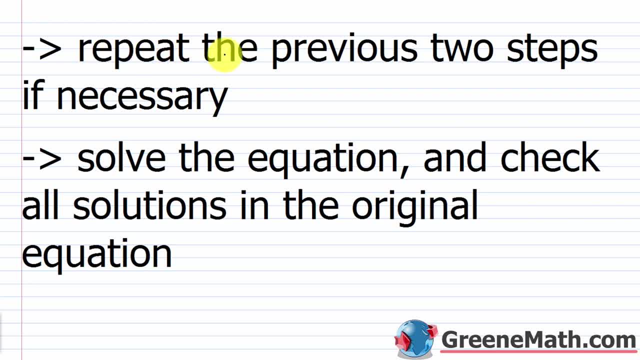 go back and isolate the radical again. So we put here, repeat the previous two steps if necessary. Sometimes you got to do it on a tougher problem, Sometimes you don't. if you get something simple, Then you're just going to solve the equation and check all solutions in the original equation. 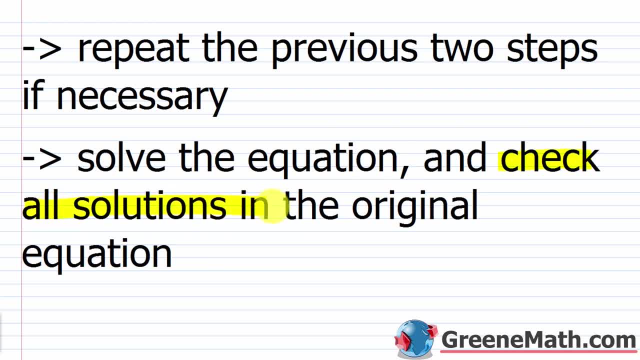 You've got to check all solutions in the original equation. okay, It's very, very important that you do that because if you don't again, you might end up reporting some answer that works in your transformed equation- okay, your new equation, but it doesn't work in the original right. 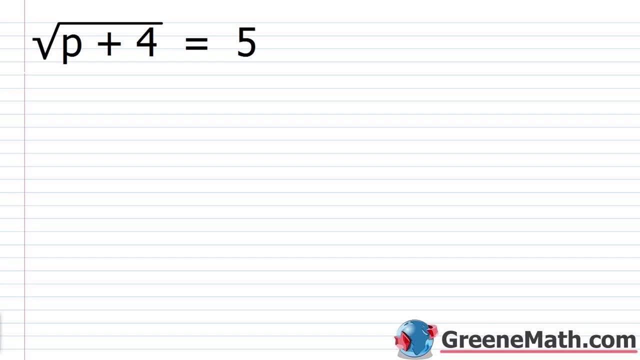 your extraneous solutions. All right, so let's start out with something very, very easy. We have that the square root of p plus 4 is equal to 5.. Now we're going to do this kind of as it sits now, and then I'm going to show you kind of with: 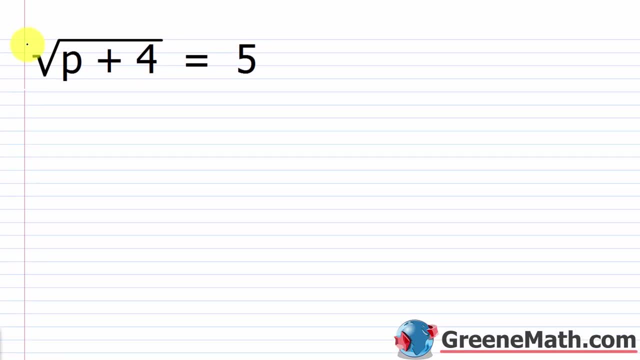 exponents so that you understand both ways. So I can again square both sides of this equation And what happens here? The squaring undoes the square root. So you can basically cancel those out And then what's left under the radical symbol, your radicand, is what's going to be. 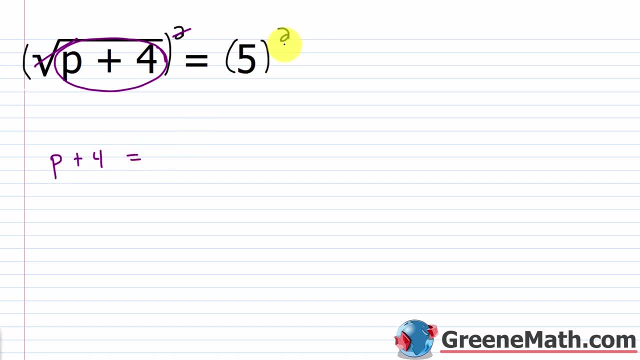 there. So you'd have: p plus 4 is equal to. if I square 5, we know we get 24.. Very, very easy equation to solve. If we subtract 4 away from each side of the equation, we'd find that p is equal to 21.. Now let me just erase this real quick. Let's think about: 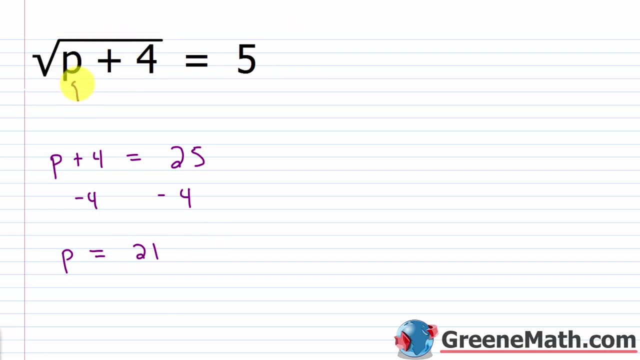 the original equation we were presented with. If we plugged in a 21 there would we have a true statement: 21 plus 4 is 25.. The square root of 25, or at least the principal square root of 25,. 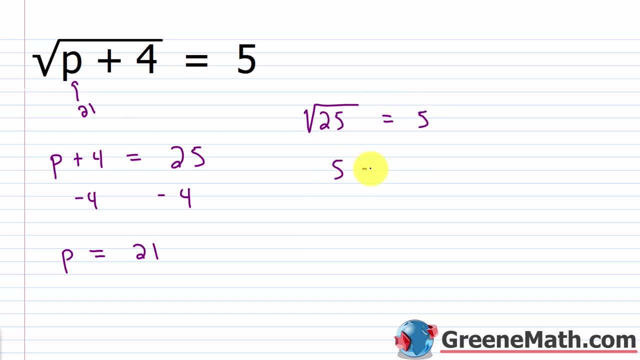 is in fact equal to 5.. So you would get: 5 is equal to 5, so this checks out. You can say your solution set contains just the element 21.. Now let me show you this using exponents, And a lot of students will see this and like: 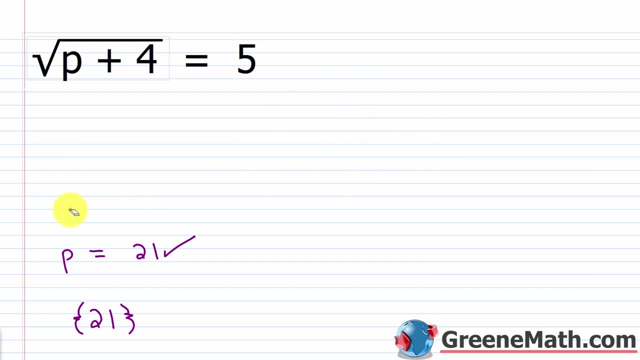 oh yeah, I get it now. This is a good way to kind of think about these. If we know already that taking the square root of something is like raising it to the power of one half, what we can do is we can say that we have p plus 4. And inside of parentheses, this whole thing is raised to the. 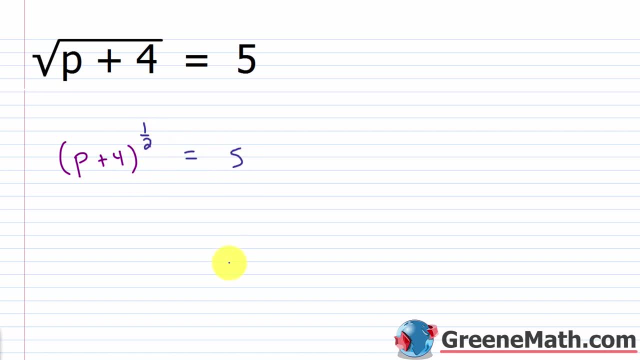 power of one half, And this equals 5.. Now, using what we know about exponents, again, if we square both sides here, let me just put this inside of brackets: and we're going to square this and we're going to. 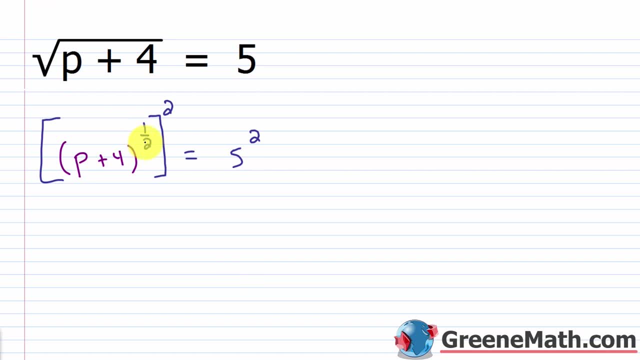 square this. What happens here? Well, we're using our power to power rule. If you're raising a power to another power, you multiply the exponents. So what is one half times 2?? Well, that's 1, these are going to cancel and it's going to be basically raised to the first power. 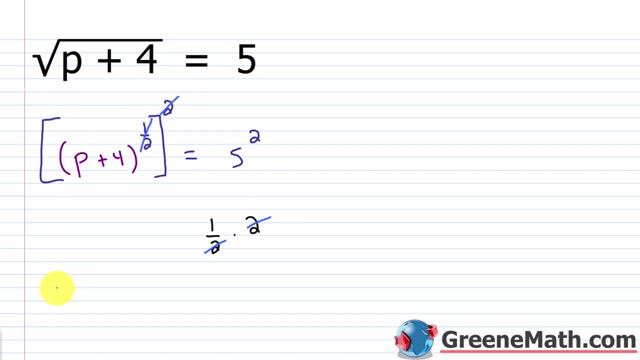 So, in other words, this would cancel with this and I'm just left with p plus 4.. So I have: p plus 4 is equal to 25. And again we solve that and we get that p is equal to 21.. So just another way to. 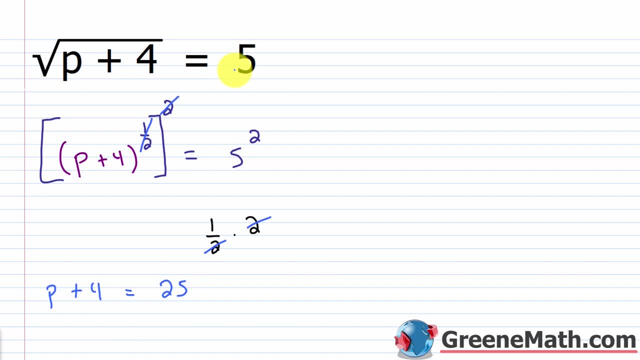 kind of think about it: if you see this on a test and you're drawing a blank on what to do, you can convert your square root into raising it to the power of one half, and then it's obvious: What do I need? I need to square it, because squaring something that's raised to the power 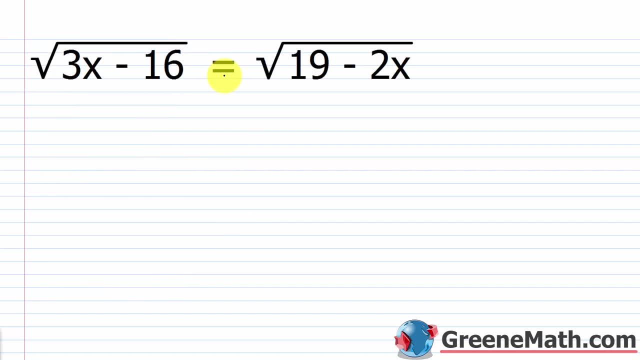 of one half would get me to an exponent of 1.. All right, for the next one I'm going to look at. the square root of 3x minus 16 is equal to the square root of 19 minus 2x. 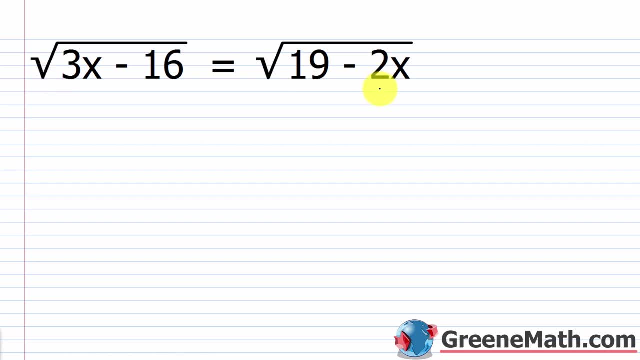 So in this case, we have a square root on one side and a square root on the other. You just square both sides. So I'm going to square this side and I'm going to square this side, And what's going to happen? Well, again, this would cancel with this. this would cancel with this. 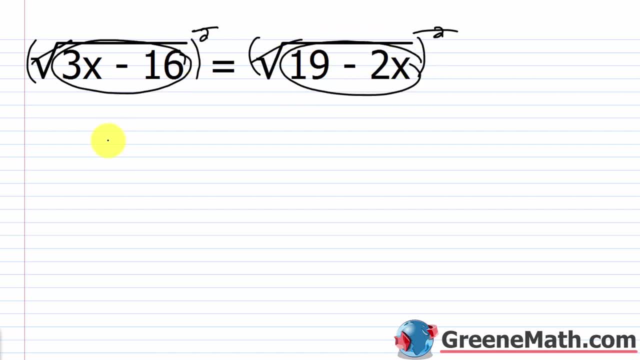 and we're left with the radicand in each case. So you basically just have: 3x minus 16 is equal to 19 minus 2x. Now we know how to solve something like this. It's very, very simple. 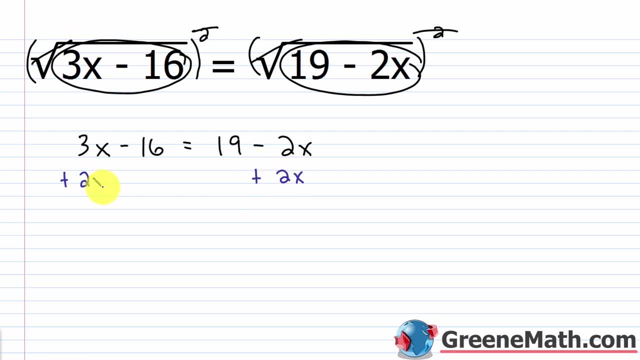 We can add 2x to each side of the equation and we can add 16 to both sides of the equation. So this is going to cancel over here and this is going to cancel over here. 3x plus 2x is 5x and this is equal to 19 plus 16 is going to give us 35.. 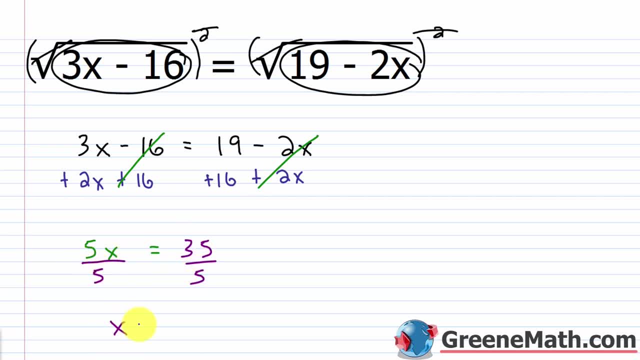 We divide both sides of the equation by 5. We get that x is equal to 6.. We get that x is equal to 7.. Again, we want to check to make sure that this is a valid solution. So let's erase all this and we're going to plug in a 7 for x here and here. 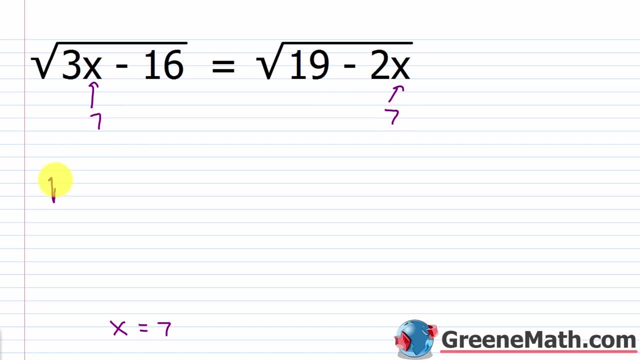 Let's see if we get the left side equal to the right. So we would have: the square root of 3 times 7 is 21.. 21 minus 16 is 5. And this is equal to 19 minus 2 times x. 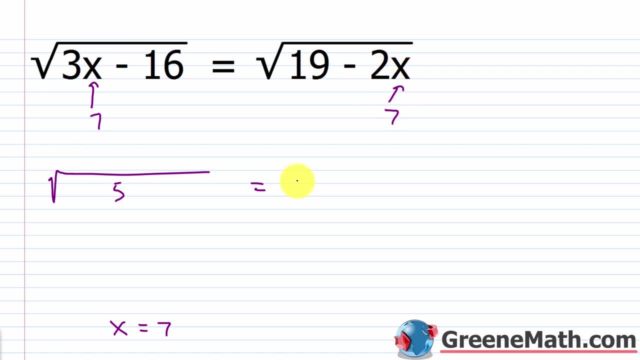 2 times 7 is 14.. 19 minus 14 is 5.. So you get the square root of 5. And 2 times the scale over here as well. Now the square root of 5 is an irrational number. 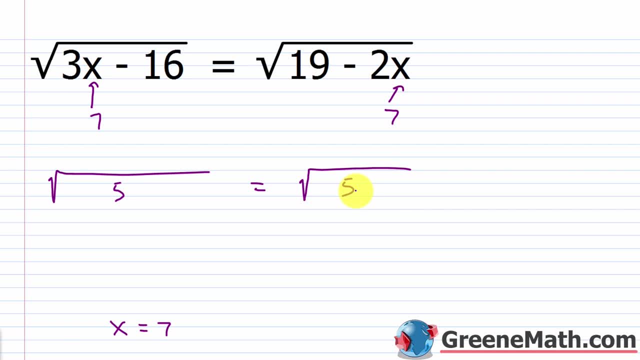 but you have, the square root of 5 equals the square root of 5.. Same thing on the left and the right. So we have a true statement here. So our solution said, for this equation just contains the element 7.. Alright, let's take a look at a harder type problem. 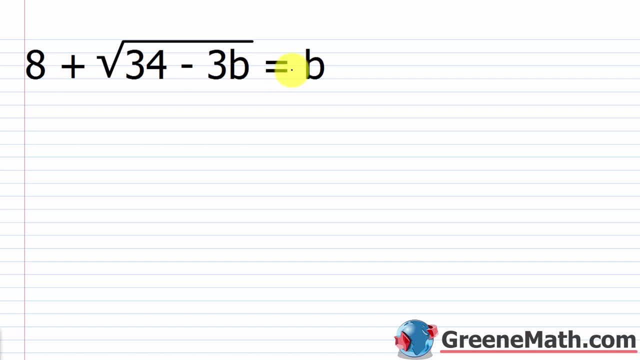 So now we have 8 plus the square root of 34 minus 3b is equal to b. What you want to do is you want to isolate your radical on one side here. So let me just subtract 8 away from each side of the equation And what's going to happen? 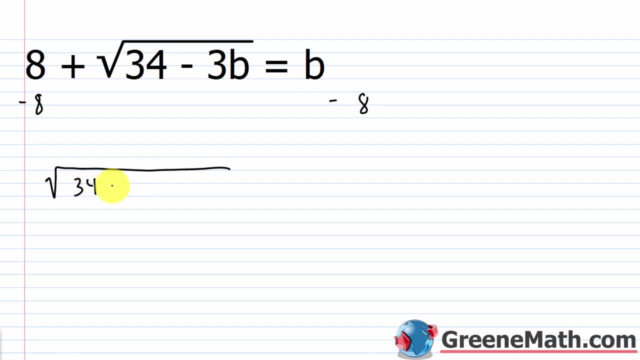 is, you'd have the square root of 34 minus 3b. This is equal to b minus 8.. Now I've isolated my radical, So all I need to do now is just square both sides. That's going to get rid of. 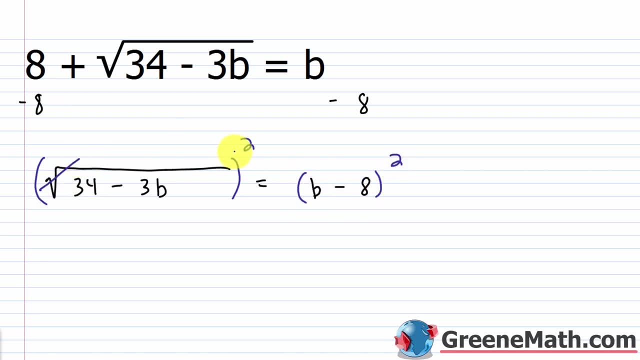 that radical, So we'll square this side as well. This will cancel with this And I just have my radical. So I just have 34 minus 3b And this is equal to Now. don't make this mistake. We talked. 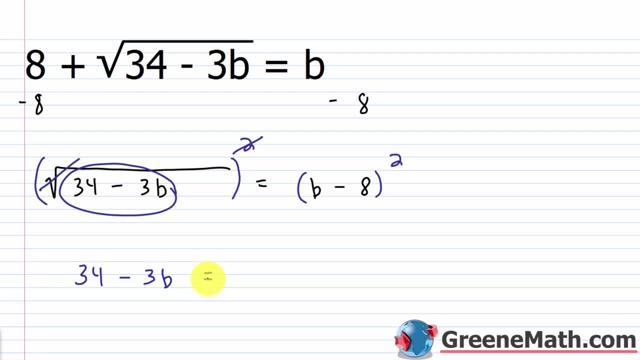 about this when we talked about polynomials. I see this all the time. You learn in polynomials and then you forget it. You go back and you say: well, this is b squared minus 8 squared. It is not. You have to expand this right Using FOIL or using your special products formula. This is: 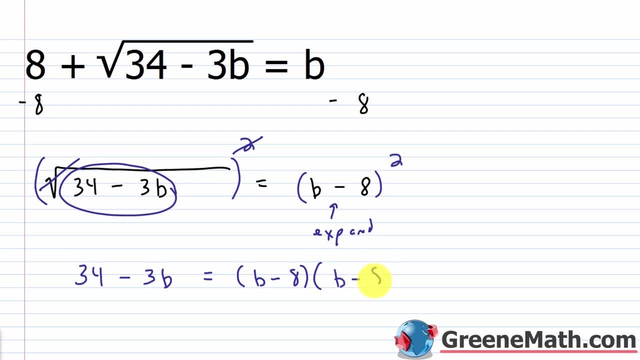 b minus 8.. Times b minus 8.. It is not b squared minus 8 squared or b squared minus 64.. That is wrong. Okay, So we know the formula for this. This is b squared minus 2 times b times 8, which is 16b. 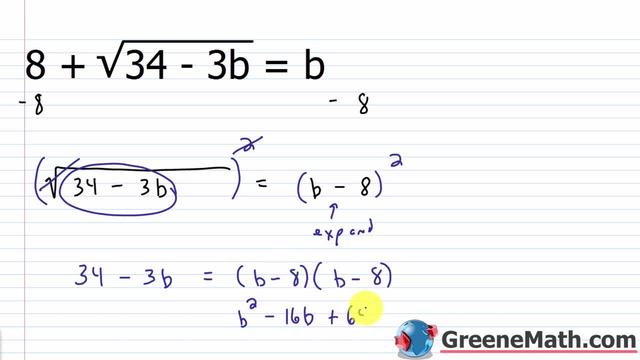 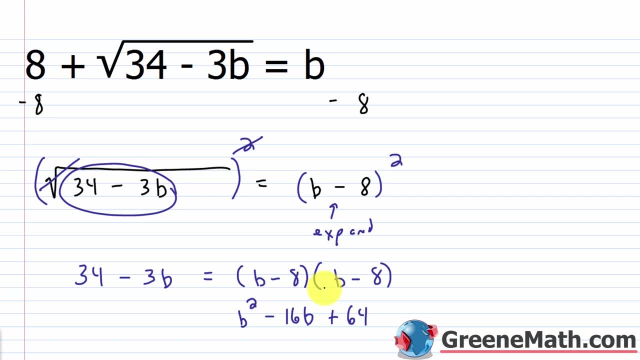 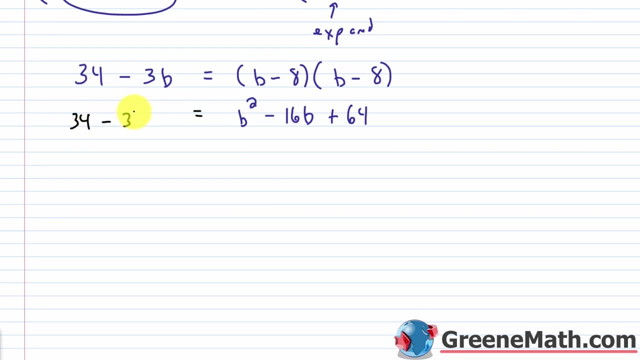 problem like this later on and you're just like: boom, I got it. You don't have to sit there and do FOIL every time. So now that we have that, let's say this is equal to 34 minus 3B, Let us. 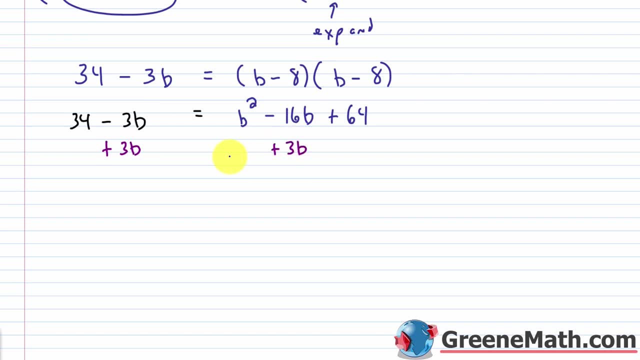 add 3B to both sides of the equation, So that's gone. And let's also subtract 34 away from each side of the equation, So that's gone. So I'm going to rewrite this. This would be zero over here, because everything's canceled. but I'm going to move all this to the left, So we would have B. 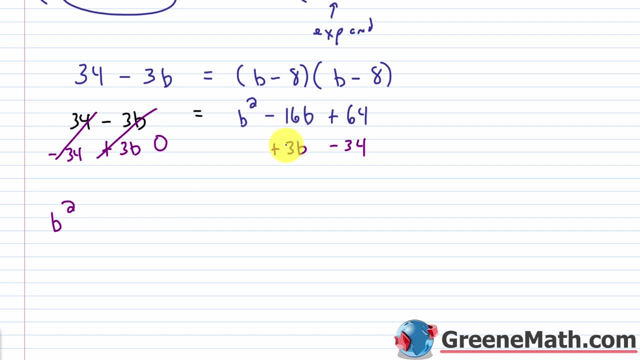 squared Negative 16B plus 3B is going to give us negative 13B, And then 64 minus 34 is 30.. So plus 30. And of course, this equals zero. And again, all I did was I just moved this to the left. 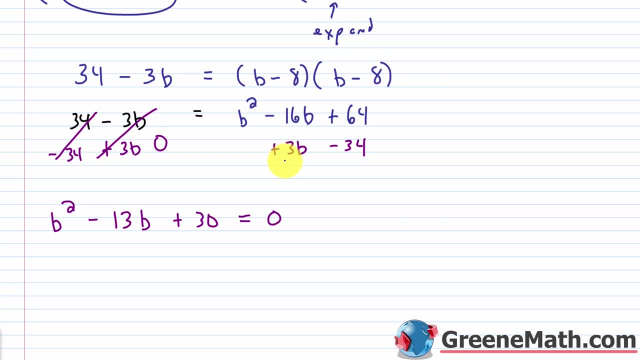 and I moved that to the right. Now we have a quadratic equation. We have in Algebra 2 so far only talked about how to solve this equation if it's factorable. So we only give you examples here where it's factorable. But again, in a few lessons we're going to start talking about. 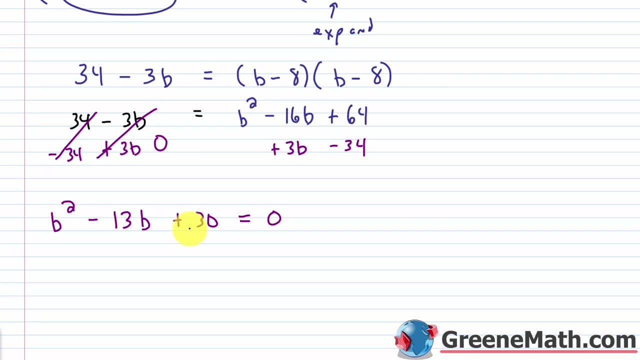 the square root, the property, the quadratic formula, completing the square things we learned back in Algebra 1 at the end. So most of you can just do this with the quadratic formula. If you want to do that, that's fine. At this point we're still doing it with factoring. So if I factor this guy, 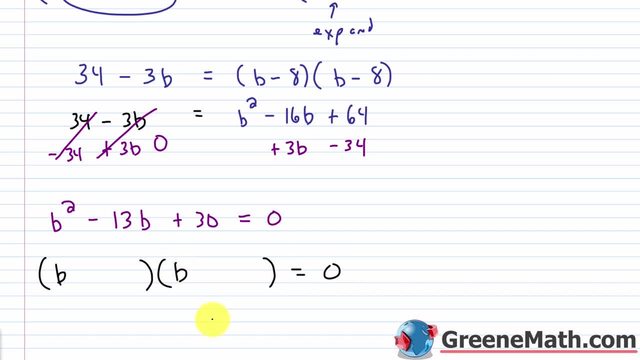 I'd have a B here and a B here, two integers whose sum is negative 13 and whose product is 30. Well, that's going to be negative 10 and negative 3. So we solve this using again our zero product property, or you could say your zero factor. 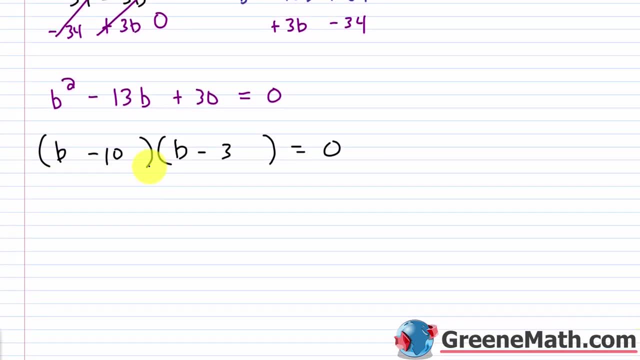 property And all you're doing is you're taking each factor- this B minus 10, that's a factor, and this B minus 3, that's a factor- and you're setting them equal to zero and you're solving So. 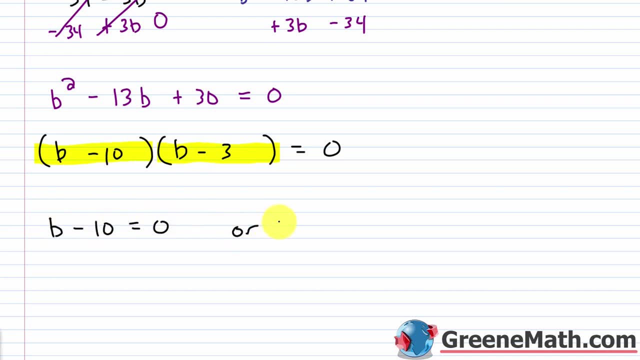 it's B minus 10 is equal to zero, or it could be true that B minus 3 is equal to zero. Either one would work as a solution. So let's add 10 to each side of the equation: We'll get B is equal to 10.. Then, or let's add 3 to each side of the equation: We'll get B is equal. 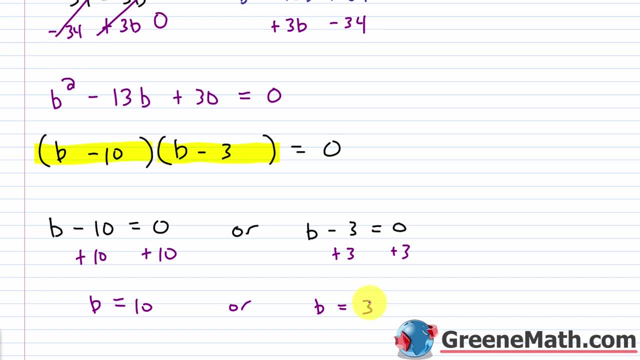 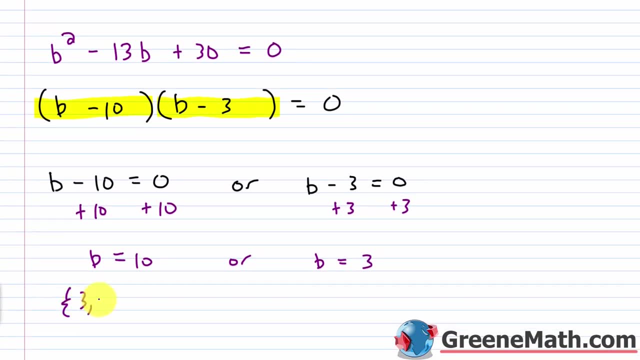 to 3.. Now these are the solutions for again our transformed equation. They're not necessarily going to work in the original, So the solution set here is 3, 10.. But let's go back up to the top. 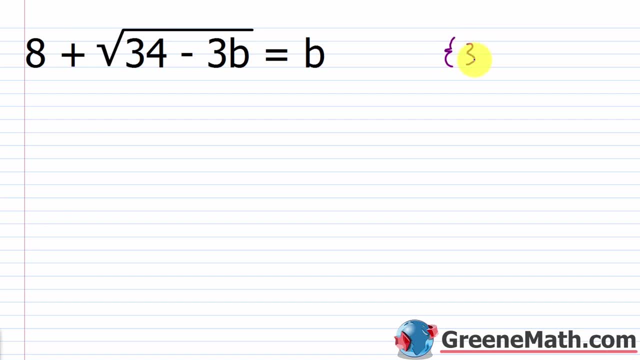 and let's see if these work out All right. so let's go ahead and check these. So if I had a 3, plugged in for B, you would get 8 plus. the square root of 34 minus 3 times 3 is 9, is equal to 3.. 34. 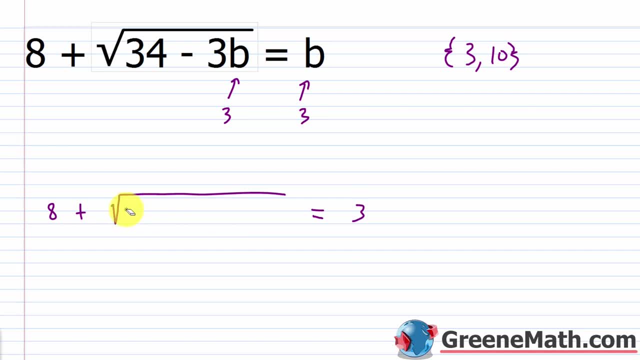 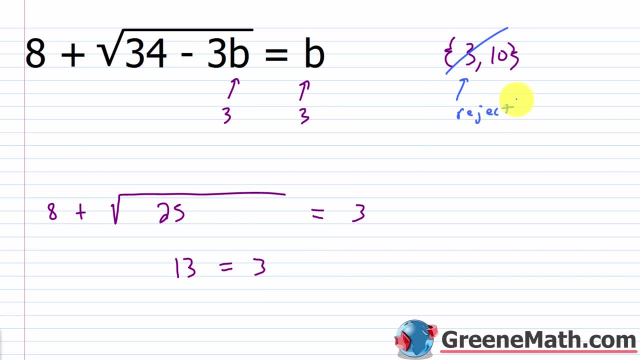 extraneous solution. It works in the transformed equation, but it does not solve or satisfy the original. Now let's try 10.. So if we plugged in 10 here and here, what would we get? We'd have 8, plus the square root of 34 minus 3 times 10 is 30, is equal to 10.. 34 minus 30 is 4.. So you'd have 8. 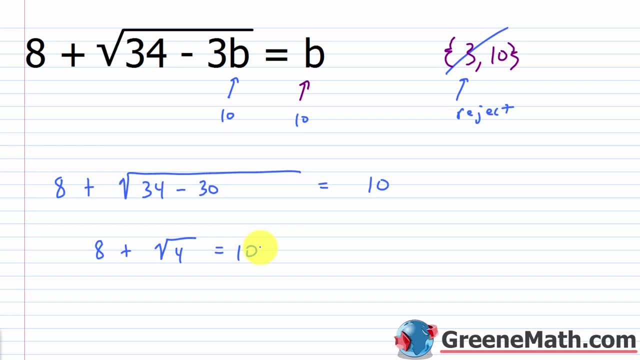 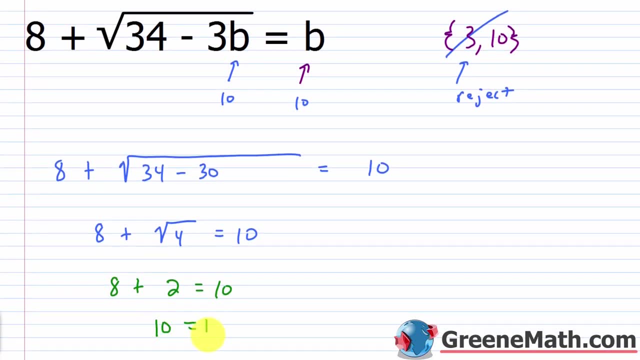 plus the square root of 4 equals 10.. You can all see at this point that this is going to work. Square root of 4 is 2.. So you'd have 8 plus 2 equals 10.. And of course, this leads to 10 equals 10.. 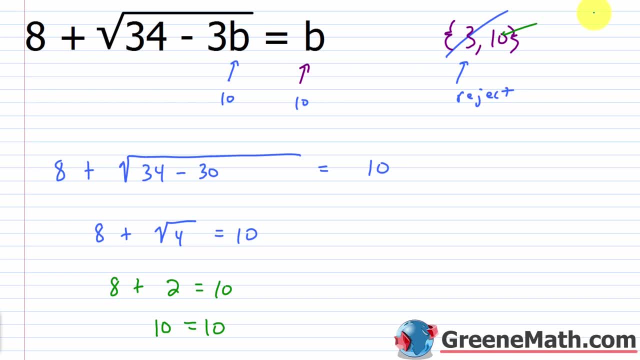 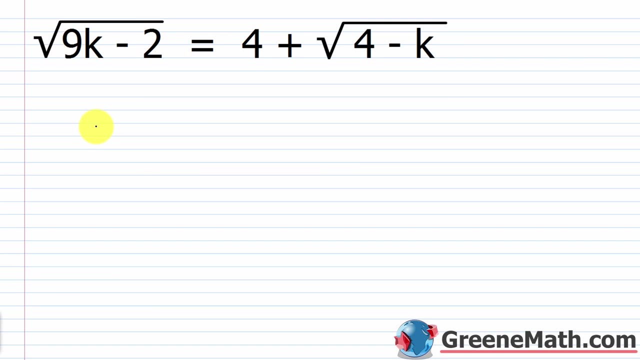 So this one does work as a solution. So the solution set for this equation is going to contain one element, just the element 10.. So you could say b is equal to 10.. Let's take a look at another one. I'm going to try one that's a little bit harder- or not harder, but just more tedious. 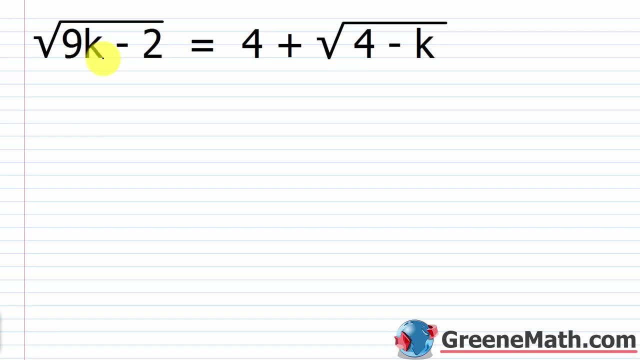 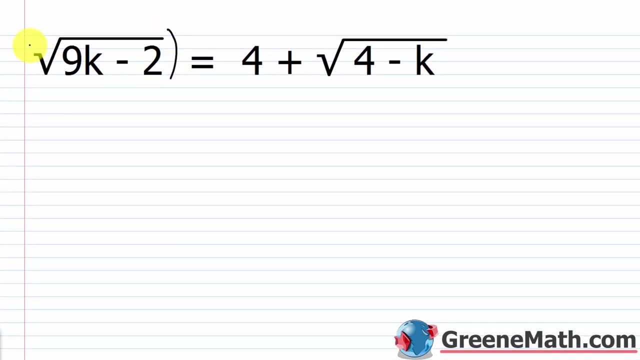 So I've got one radical that's isolated on one side. On the other side, I've got a radical plus a number. So what we want to do is again just square both sides. And you're not going to be radical free the first time you do this here. So if I square this side, 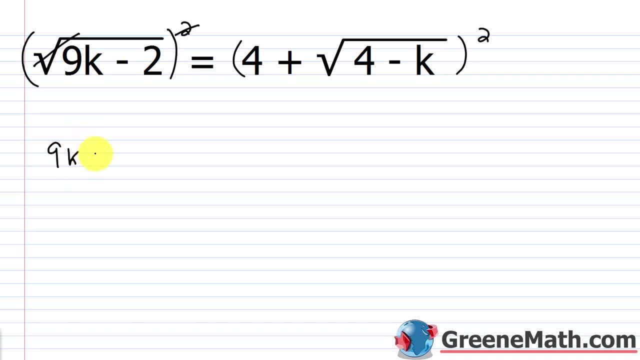 this will cancel with this And we'll have the radicand, which is 9k minus 2.. Then this is equal to Over. here I'm going to go ahead and use my special products formula. You have to be just very careful about this. This right here, you're going to treat it just like you would. 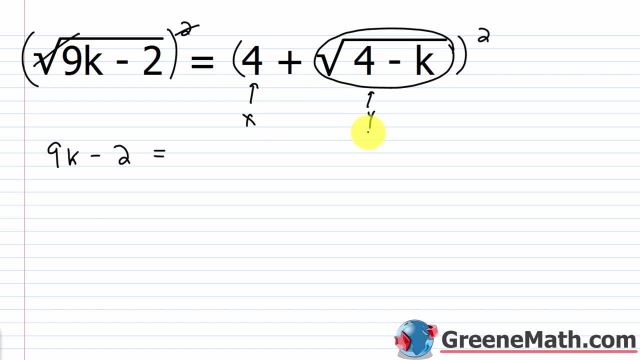 let's say this is x and this is y. You'll see what I mean. So for that formula the first guy gets squared, So it's 4 squared plus 2 times the first guy. times the second guy, 2 times 4 is 8. 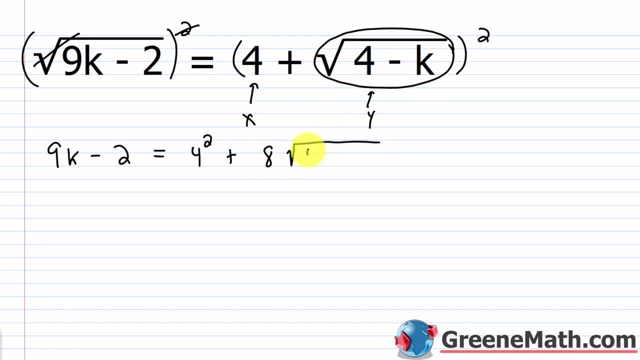 times the second guy, which is the square root of 4 minus k, Then plus, you've got the last guy squared. So if I squared the square root of 4 minus k, I'd be left with 4 minus k. All right, So now. 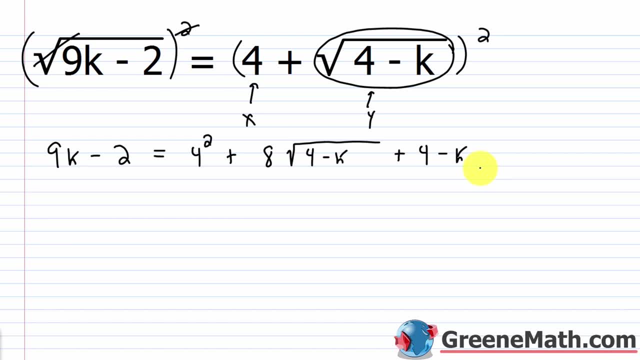 that we have that. we want to do some simplifying. The easiest thing is 4 squared. we know that's 16.. Let's go ahead and just write that, And then 16 plus 4 is 20.. So we could say that we have 9k. 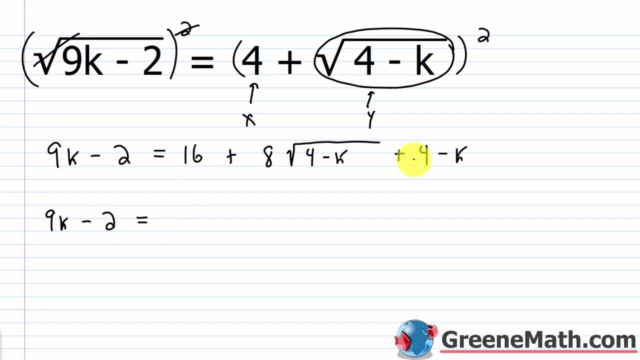 minus 2 is equal to again 16 plus 4 is 20, plus 8 times the square root of 4 minus k and then minus. Now we know that we can add k to both sides of the equation. 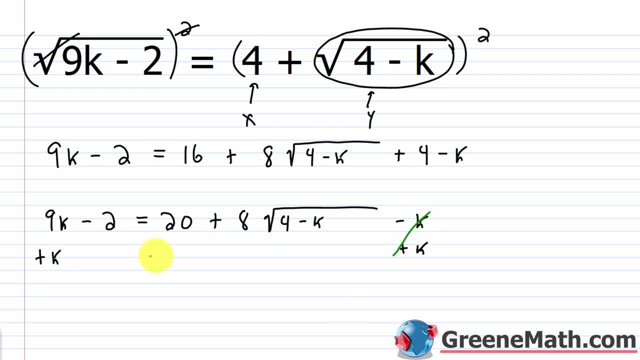 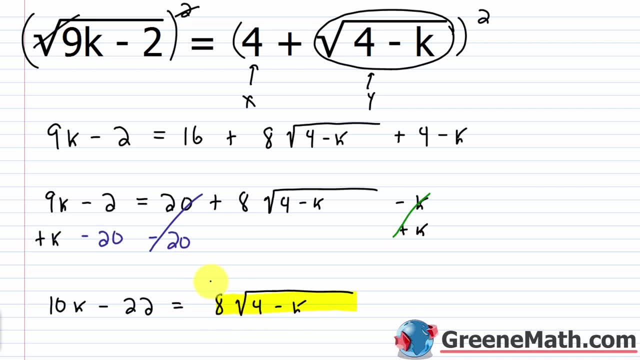 Is everything divisible by 8 here? Because if I divide it by 8, I could get rid of that out in front. But 10 is not divisible by 8, and 22 is not divisible by 8.. So I wouldn't do that here. 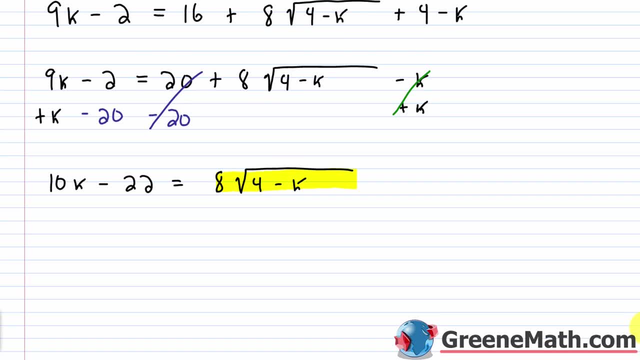 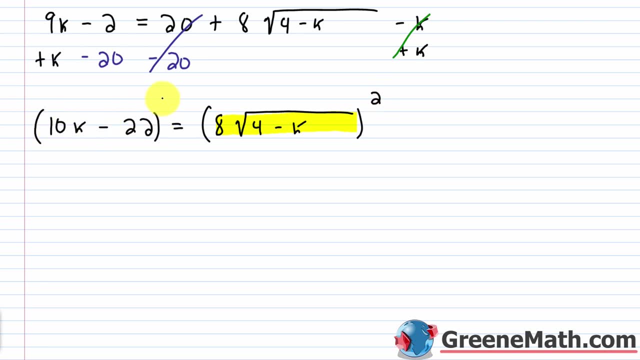 Okay, You can do it, but I think it would cause more work, because you're going to end up with some kind of nasty fractions to work with. So let's go ahead and just square both sides of the equation. And what are we going to get Over here? we're going to use our special products formula. 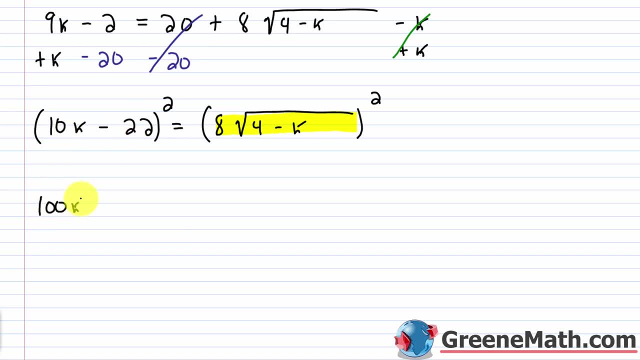 We know we would square 10k, so that's 100k squared Minus 2 times. this times this: 2 times 10 is 20.. 20 times 22 is 440.. And then, of course, times k. 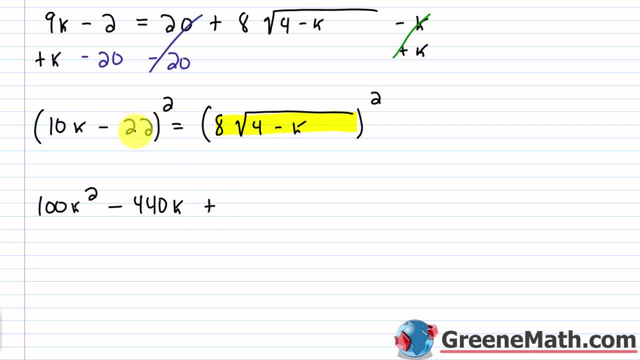 Then the last guy is: plus this guy squared, 22 squared is 484.. Then this is equal. to Remember, this is multiplication here. So it's kind of like you're saying you have 8 squared multiplied by the square root of 4 minus k squared. You just got to make sure that you. 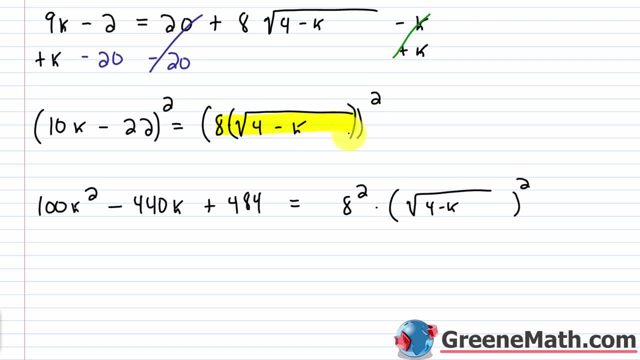 raise both of these to the point where you get the square root of 4 minus k squared. So in other words, you can kind of put this inside of parentheses and say 8, again will be squared, And then this guy inside of parentheses, the square root of 4 minus k, that's raised to the 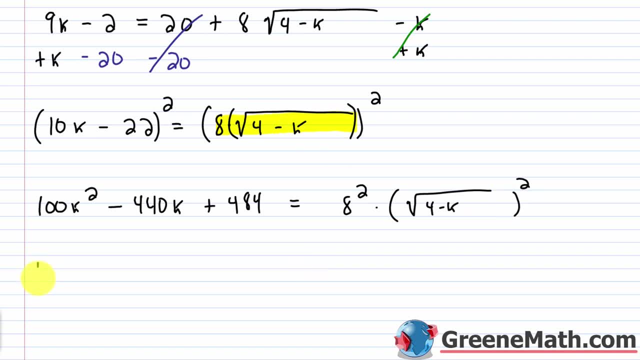 power of 2 as well. All right, So let's continue simplifying. We've got 100k squared minus 440k plus 484 is equal to 8, squared, of course, is 64.. And then the square root of 4 minus k squared. 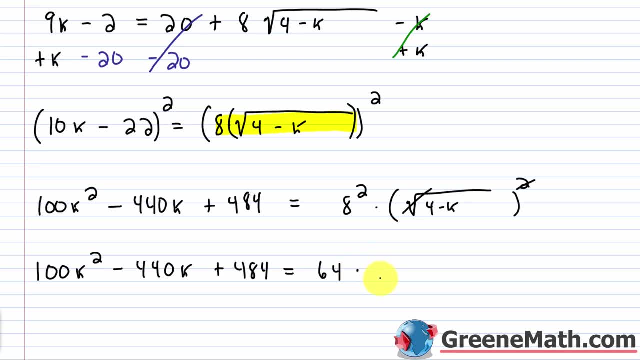 again, this cancels with this. So you're going to have: this: is multiplied by, okay, 4 minus k. And this has to be in parentheses because again this guy right here, this 8 squared, is multiplying this whole thing. Okay, So don't make the mistake of just saying. 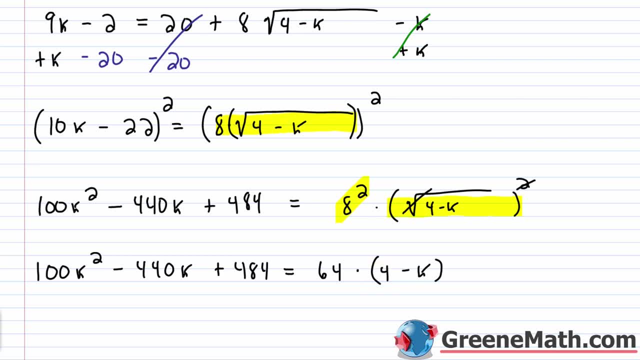 oh, we've got 64 times 4.. That's not going to work. Okay, You've got to multiply it by the 4 and by the negative k, All right, So let's continue here. So we've got 64 times 4,. 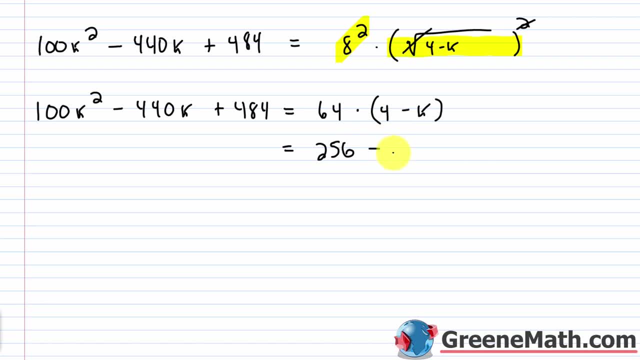 which is 256, and then minus 64 times k, which is just 64k. So over here we still have our 100k squared minus 440k plus 484.. All right, So let's add 64k to each side of the equation. 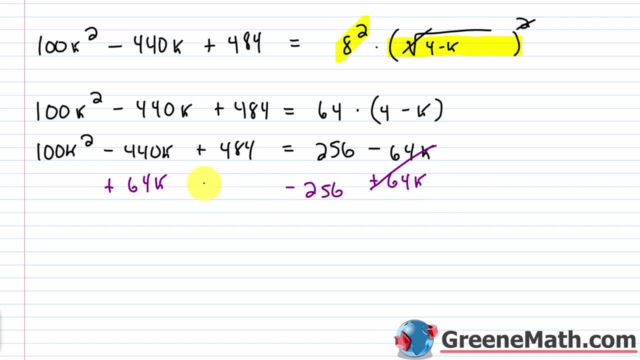 That'll cancel. Let's subtract 256 from each side of the equation. That'll cancel. So we'll end up with 100k squared and then negative 440k. plus 64k is negative 376k, And then 484 minus 256 will be plus 284k. 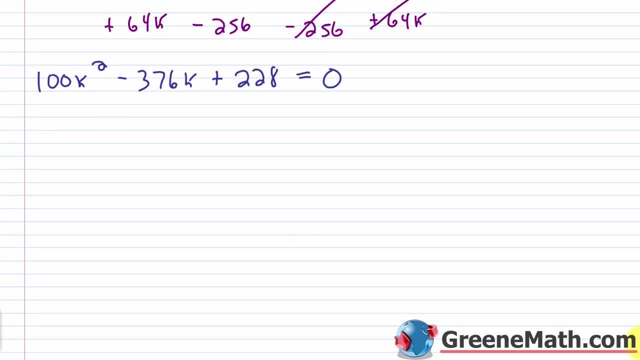 228.. And this equals 0.. Now again, so far in algebra we've only talked about kind of doing these problems, these quadratic equations, with factoring. The first thing you would notice is that everything is divisible by 2.. 100 is divisible by 2.. 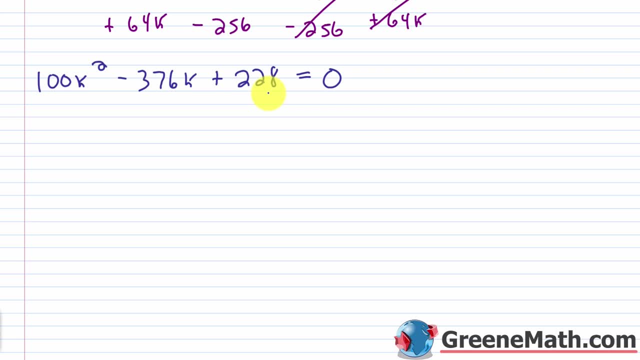 So is negative 376.. So is 228.. Now the other thing is that everything is divisible by 4.. So a cool little trick to work with smaller numbers. we can divide both sides of this equation by 4.. If I divide 0 by 4, I just get 0.. So what does that matter? right? So this will still be 0.. 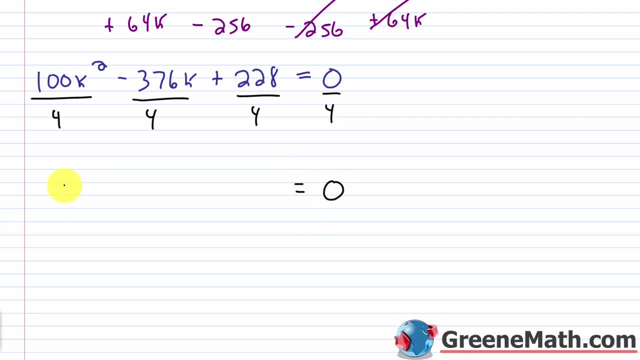 If I take 100 and divide by 4, I get 25.. So this would be 25k squared, then minus 376, divided by 4 is 94. So this would be minus 94k And then plus 228 divided by 4 is 57.. 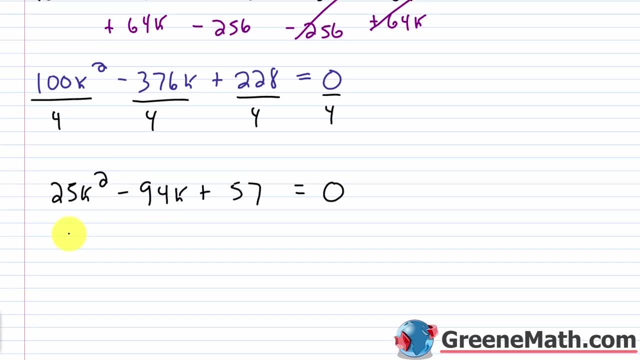 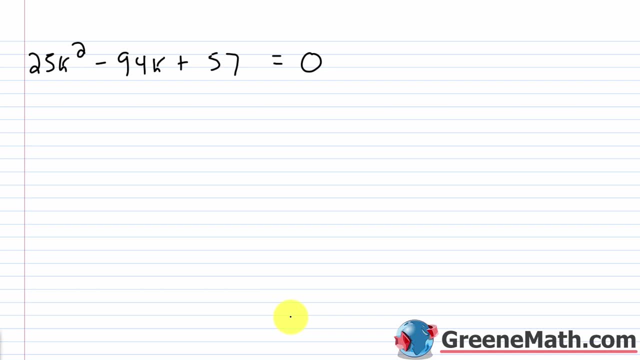 You can use the quadratic form if you want. We haven't gotten to that yet, So we're going to solve this by factoring here. So I want two integers whose sum is negative 94 and whose product is 25 times 57, which is 1,425.. So if you factor this again, we know this came from 25 times. 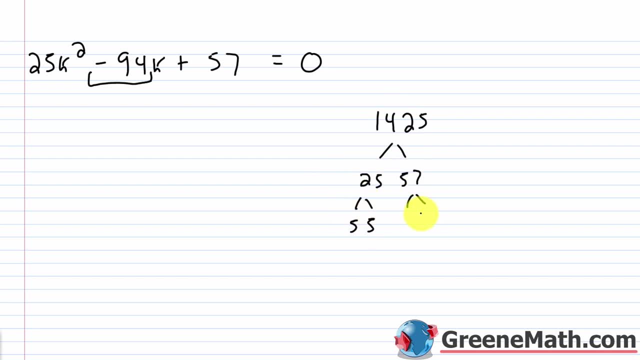 57.. This is 5 times 5.. This is 19 times 3.. So right away you know that you want two negatives, right? Two negatives. If you sum to a negative, two negatives multiply to be a positive. So thinking about that, 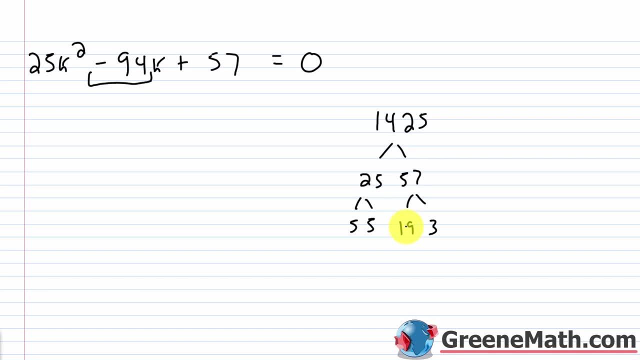 5 times 5 times 3 is 75. So 25 times 3 is 75.. 75 plus 19 is 94.. Just got to work out the signs, right. You just want all that to be negative. So what you would want is two integers negative 75. 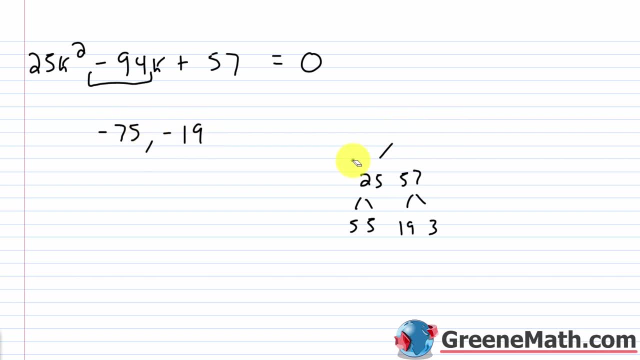 and negative 19. So we're going to use those two to rewrite that middle term. Okay, So we'll have 25k squared minus 75k, minus 19k plus 57 equals zero From the first group. here we can pull out a. 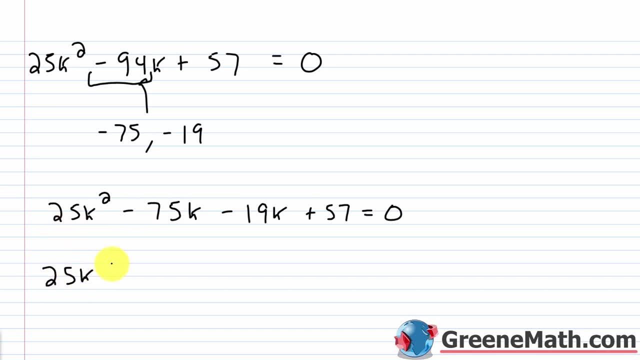 25k, So we'll pull that out. So inside we'll be left with k minus 3.. From the second group here, because the signs are in a different order: right, This is plus, this is minus, this is minus. 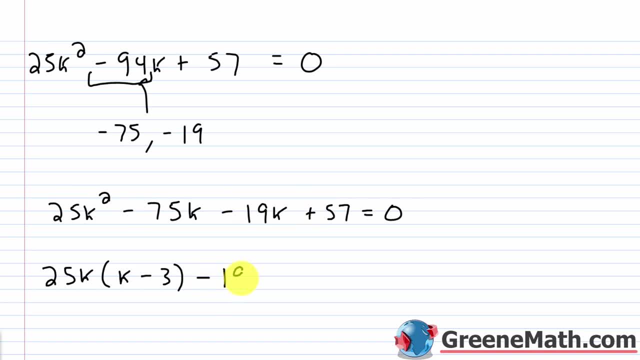 this is plus. We're going to pull out a negative 19, and that'll leave us with k minus 3 inside, And so we have this common binomial factor, this k minus 3.. That can be factored out, So let's go ahead and take that. 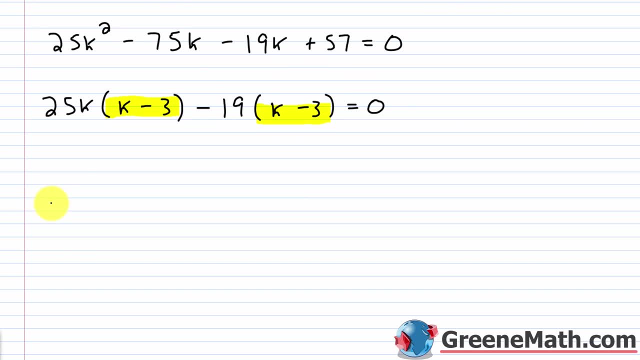 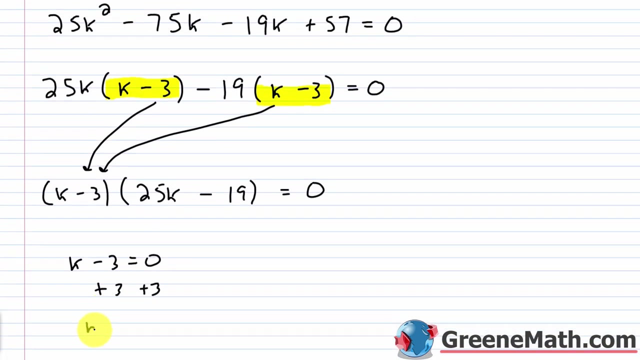 out And what we're going to have is we'll have k minus 3.. Again, we're factoring that out. Times what's left is going to be 25k minus 19, and this equals zero. Again, zero factor property. So you've got k minus 3 equals zero. Add 3 to each side. You get k. 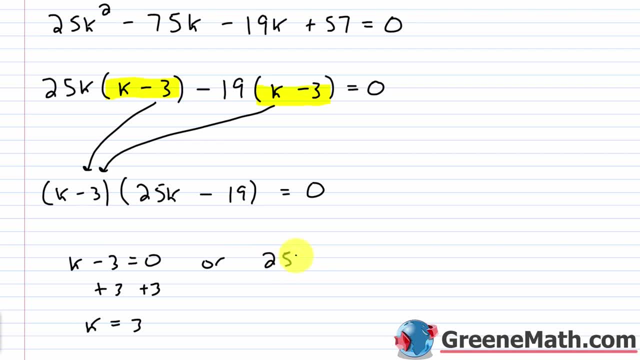 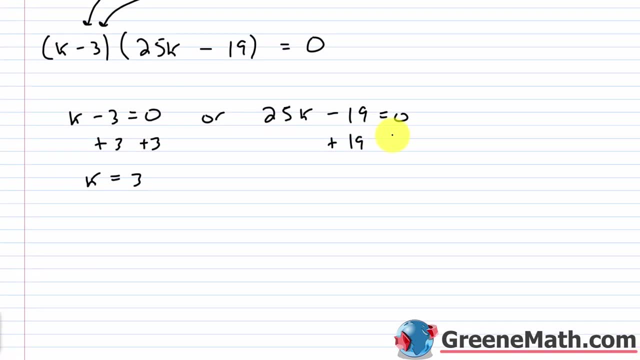 equals 3.. Or 25k minus 19 equals zero. Add 19 to each side of the equation, You'll get 25k is equal to 19.. Divide both sides by 25, and you'll get that k is equal to 19.. So we're going to get k minus 19. 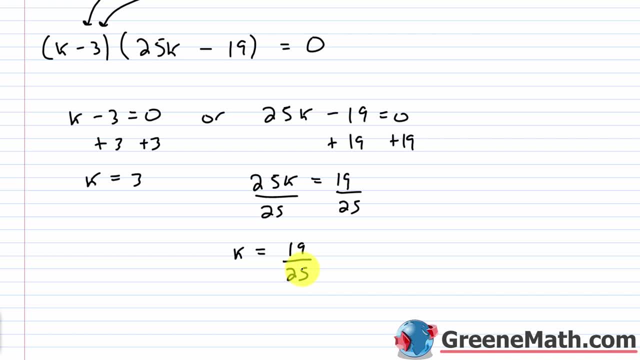 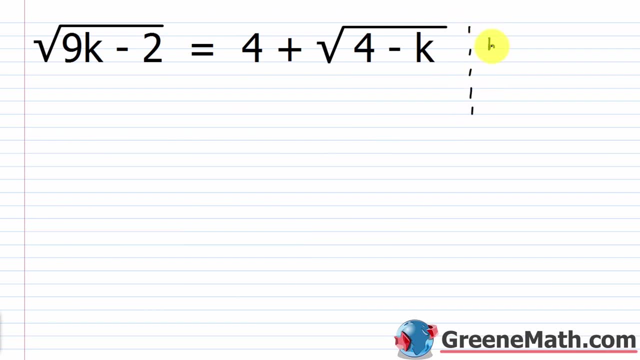 twenty-fifths. We need to check both of these in the original equation. So k equals 3 or k equals 19, twenty-fifths. All right, so let's check again. You want to check? k equals 3 or k equals 19? 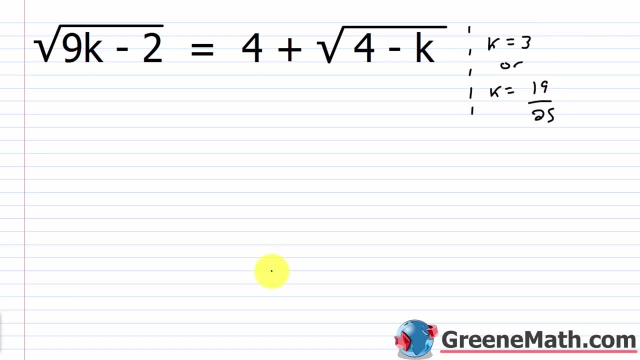 twenty-fifths. All right, let's do 3 first. That one's easier to do. So if you plug in a 3 here and here, you would have the square root of 9 times 3, which is 27.. Let me just go ahead and 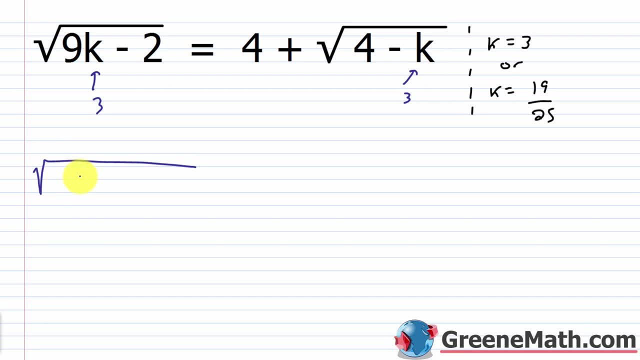 write that 27 minus 2, which is 25.. So square root of 25 is equal to 4 plus the square root of 4 minus 3 is 1.. So it's a square root of 1.. Square root of 25 is 5 equals 4 plus square root of 1. 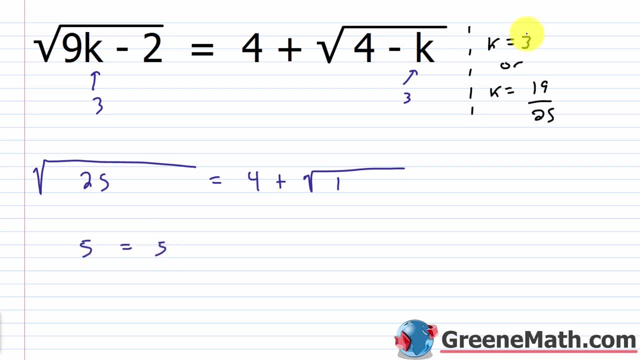 is 1.. So 4 plus 1 is 5.. 5 equals 5.. So yeah, this one's going to check out Now the other guy over there. that's going to be much more tedious. But again, these you have to check them. so it's not something you could just kind of skip. 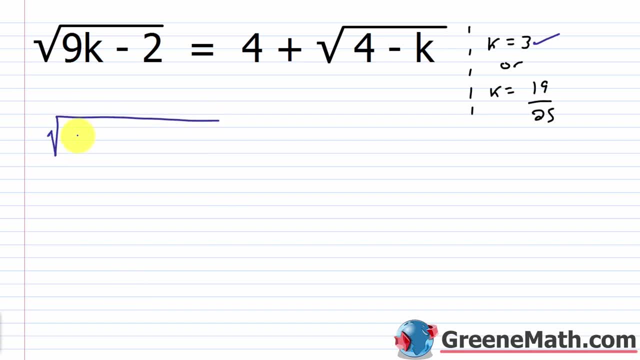 through. So we'd have the square root of 9 multiplied by 19 25ths minus 2.. This should be equal to 4 plus the square root of 4 minus 19 25ths. Alright, so over here, 9 times 19 is 171.. So this would be the square root of 171. 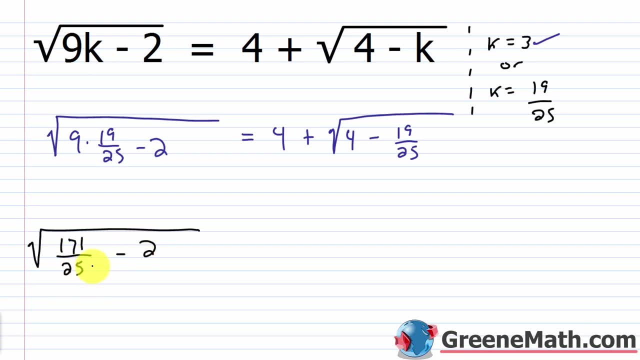 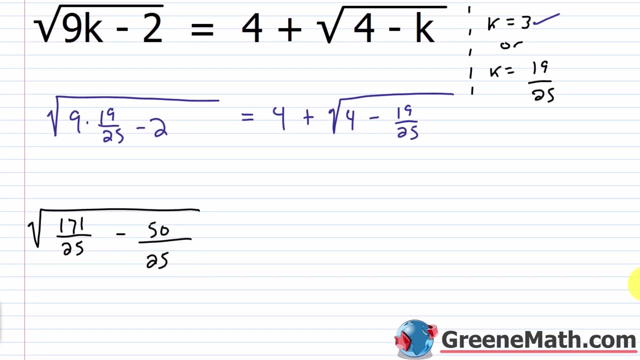 over 25, then minus 2.. Now I want a common denominator going, so I'm just going to multiply this by 25 over 25.. So you might as well just say this is 50 over 25.. So if I did this operation, 171 minus 50 would be what That would be. 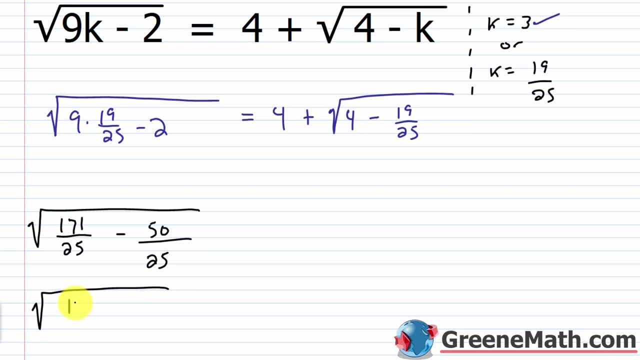 121.. So this would be the square root of 121 over 25. and then we know the square root of 121 is 11.. We know the square root of 25 is 5.. So you might as well just write: this is 11.. 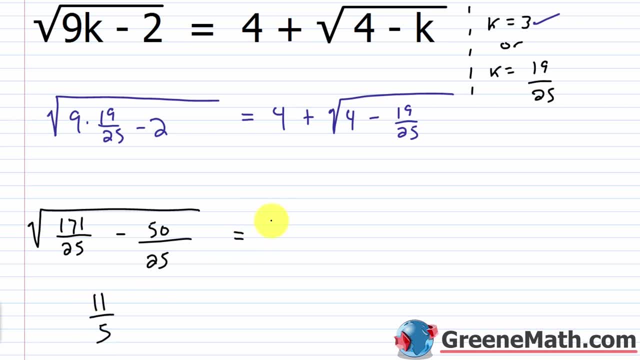 So this is equal to: you've got 4 plus the square root of 4 minus 19 over 25.. Again, if I get a common denominator going, multiply this by 25 over 25.. It's essentially 100 minus 19, which is 81. So this would be the square root of 81 over 25.. We know the square root. 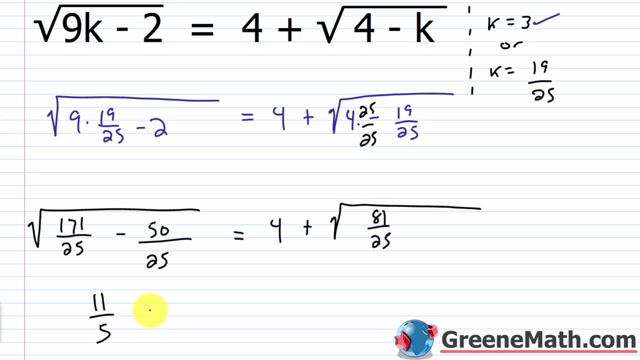 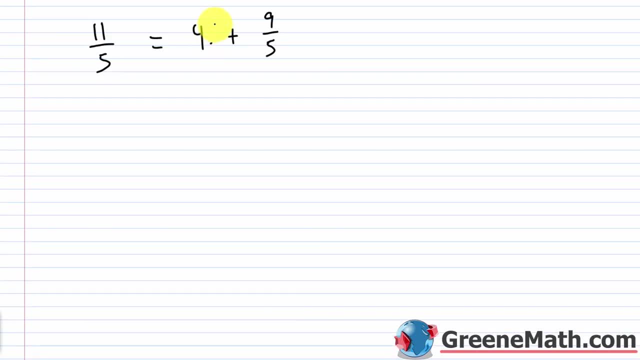 of 81 is 9.. We know the square root of 25 is 5.. So this should be equal to 4 plus 9 5ths. So get a common denominator going here. Let's multiply this by 5 over 5. You'll get. 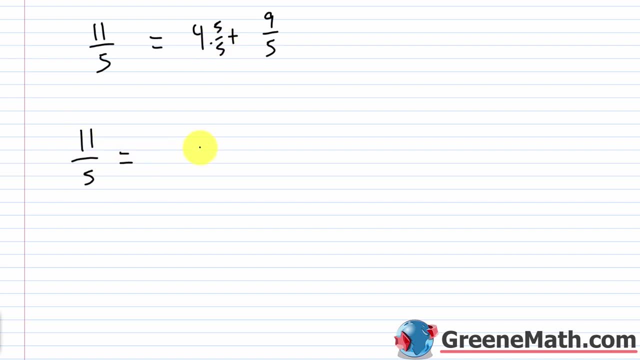 11 5ths is equal to 4 times 5 is 20.. So you end up with 20 plus 9, which is 29 over 5.. So 11 5ths does not equal 29 5ths. That's false, So we have to reject that solution. 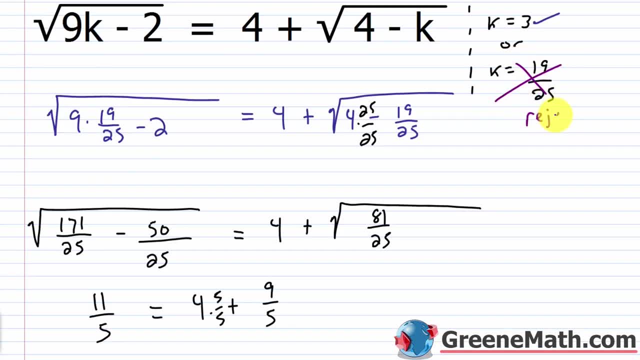 So let's go back up and let's reject this guy, because it doesn't work in the original equation. So your only solution here is going to be that k is equal to 3.. We're again using a solution set notation. You just put 3 as your only element, And so again, that's why. 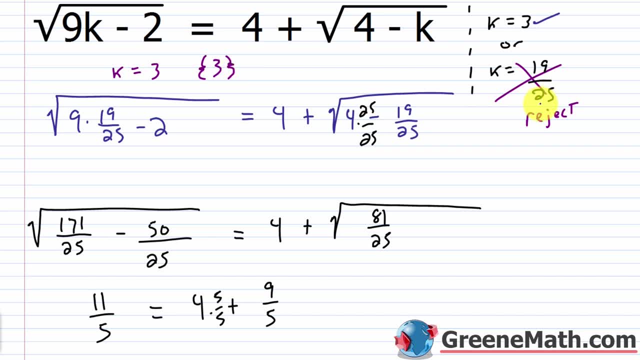 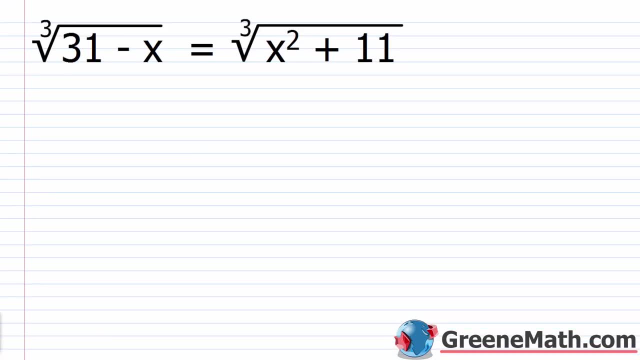 it's so important to check these, And I know you get some of these that are going to be really, really tedious, but they throw those in there just so you get some good practice. All right, let's take a look at one that's a cube root now. So we have the cube root. 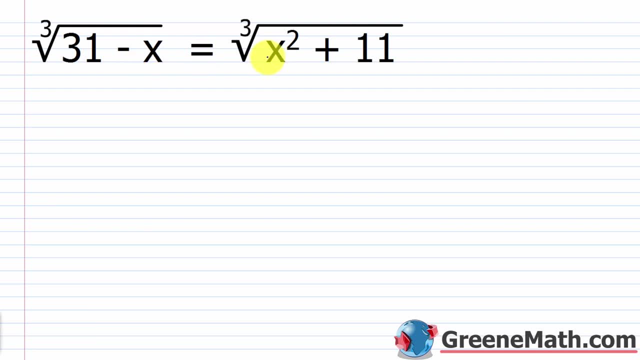 of 31 minus x is equal to the cube root of x squared plus 11.. So with this one it's very easy. Again, if I have a cube root, I want to raise everything to the third power, or I want to cube it. So what happens is this cancels with this. Right, you can think about this. 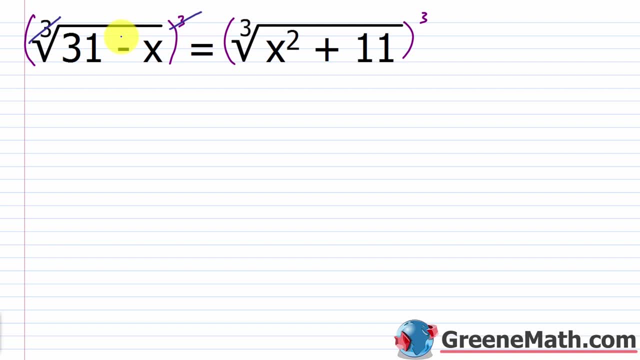 as I have the 1- 3rd power raised to the third power, 1 3rd times 3 is 1.. All right, so they just cancel each other out. I'm left with just my radicand, which is 31 minus x Over. 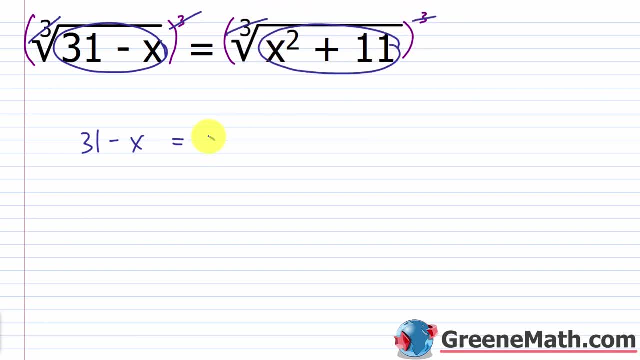 here same thing. This cancels. with this, I'm left with my radicand, which is x squared plus 11.. And so all we really need to do here, let's add x to each side And let's subtract 31 away from each side. 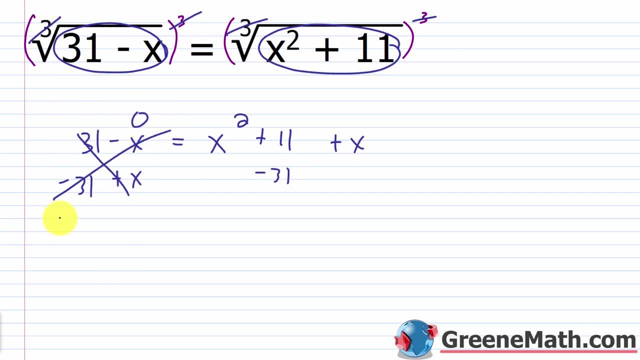 That'll cancel and become 0. You will have that 0 is equal to x squared plus x. 11 minus 31 is going to give us negative 20.. And we could rewrite this as: x squared plus x minus 20 is equal to 0.. Now again, we're going to solve this using our zero factor property. 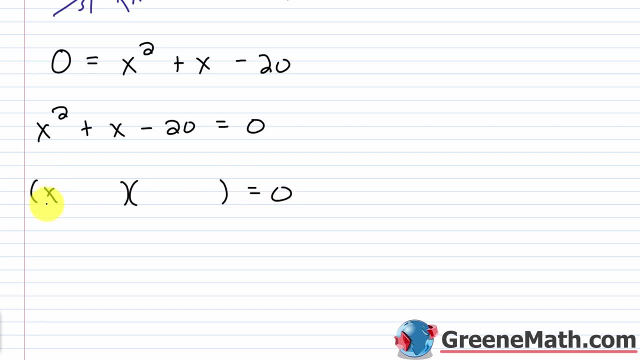 So let's factor this guy and see what we can get. I know this is x and this is x. Two integers whose sum is 1 and whose product is negative: 20 would be positive 5 and negative 4.. Now we'll set each factor equal to 0. So you'll have x plus 5 equals 0, or x minus 4 is equal. 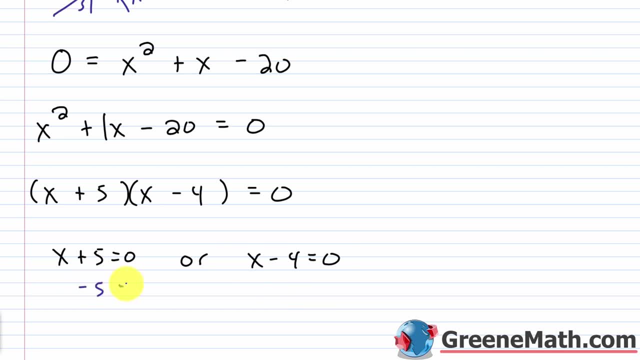 to 0.. If we then subtract 5 away from each side of the equation, we'll get x is equal to negative 5.. Over here, if we add 4 to each side of the equation, we'll get that x is equal to 4.. 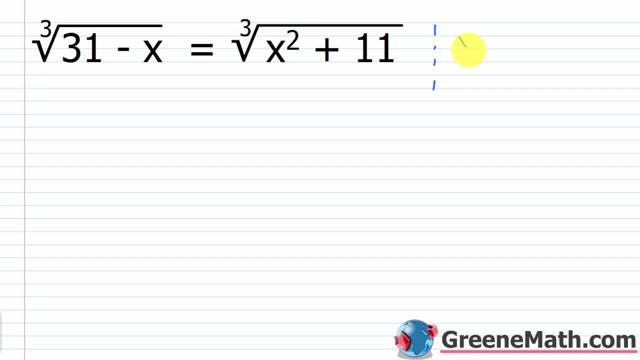 Alright. so the two solutions we found were x equals negative 5 and then x equals positive 4.. Just going to plug them in like we have been. So if I plug in a 4 there and there, what will we get? We'll have the cube root of 31 minus 4, which is 27, is equal to the. 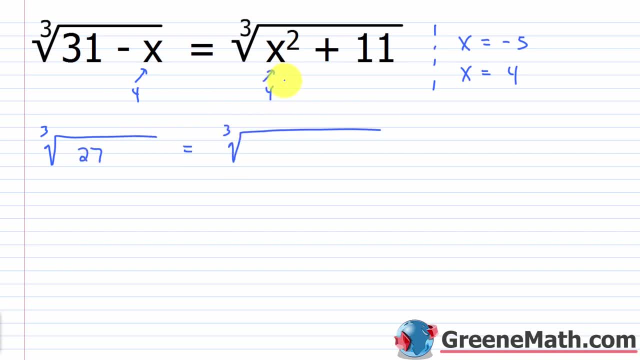 cube root of 4 squared, which is 16 plus 11, which is 27.. So obviously, the cube root of 27 does equal the cube root of 27.. This is basically 3 equals 3.. So this guy's going to check out. The next one we want to try is negative 5.. Okay, negative 5.. So let's plug. 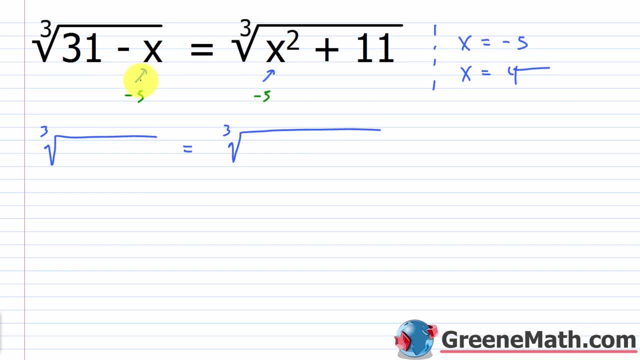 that in there and then there. So 31 minus a negative 5 is like 31 plus 5.. 31 plus 5 is 36.. So you'd have the cube root of 36.. Then over here you have to be careful because you have negative. 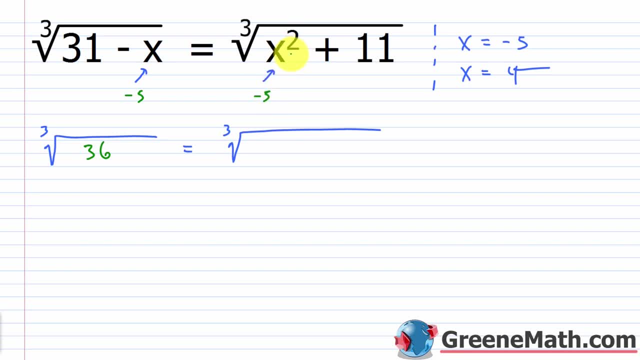 5 squared Negative 5 squared is 25.. 25 plus 11 is 36 as well. So we'd have the cube root of 36 equals the cube root of 36.. Same value on each side, So this solution works as well. So your. 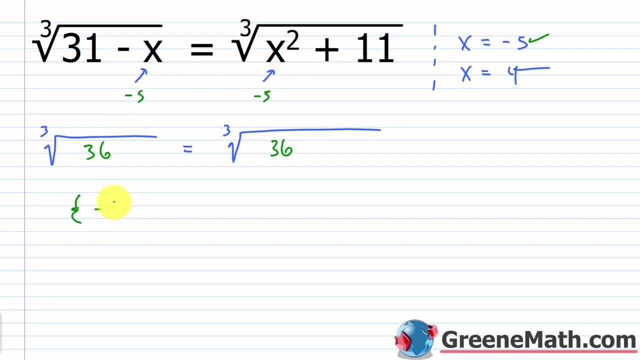 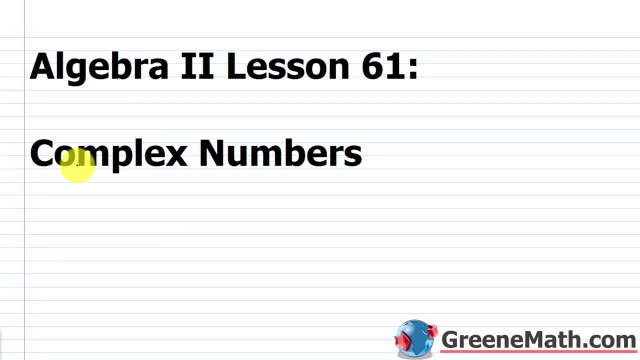 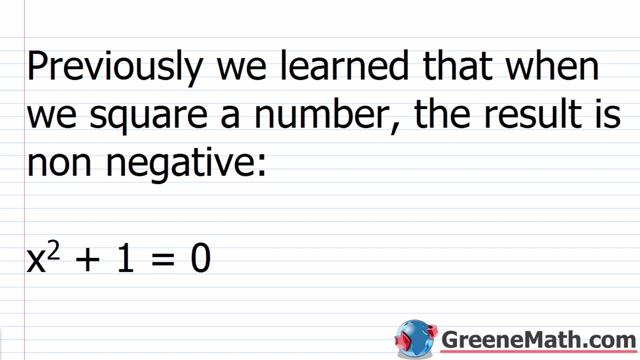 solution set for this equation contains two elements. We have negative 5 and 4.. Hello and welcome to Algebra 2, Lesson 61.. In this video, we're going to learn about complex numbers, So the purpose of this lesson is to deal with the situation where you have to take the square root of some negative value And 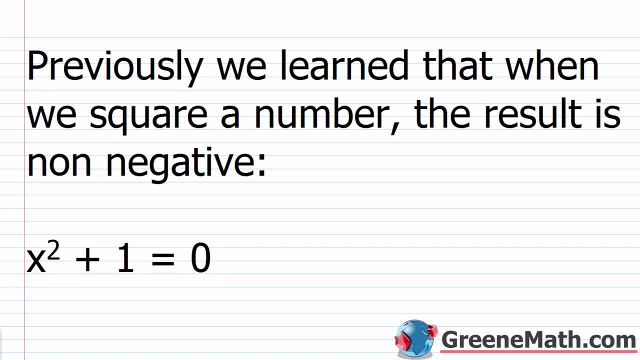 this comes up immediately in the next lesson when we start working with quadratic equations again. A lot of you will recall back in Algebra 1, we ended our course by learning how to solve quadratic equations using the quadratic formula. But it doesn't matter what method you're using. 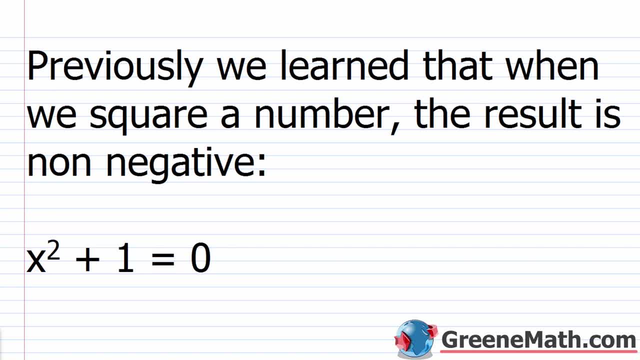 if you're required to take the square root of a negative value from your first problem When you fled the lesson where you learn about complex numbers, you basically have to just stop the problem and say, Hey, there's no real solution. So let's talk a little bit more about why there's no real solution. Previously we learned that when 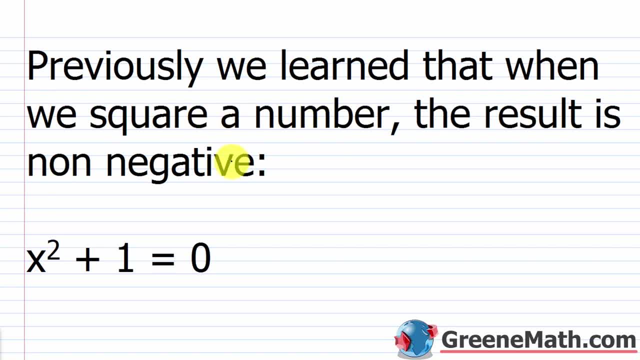 we square a number, the result is non negative. So we all know if we take something like negative 1 and we square it, we're going to end up with 1.. Right, positive, 1.. If we took negative 4 and squared, 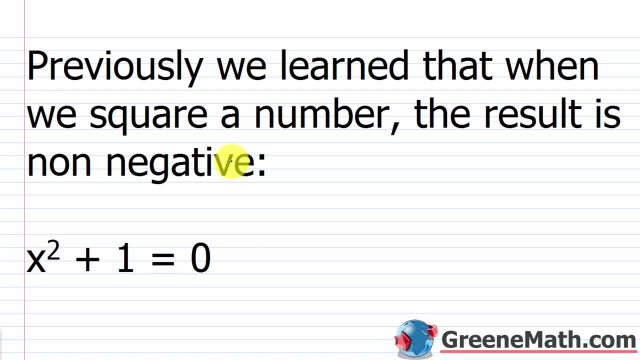 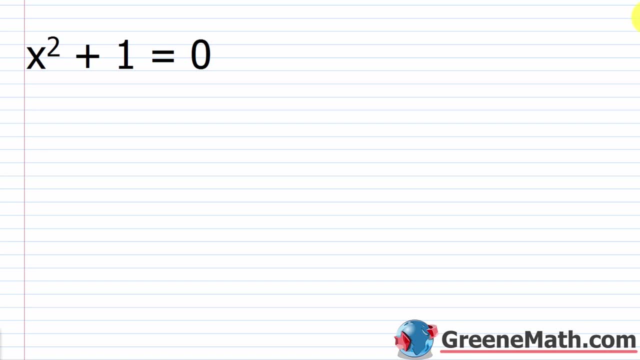 we're gonna end up with positive 16.. so on and so forth. The only thing you can have as a result of squaring something in the real number system is either zero or some positive value, but you'll never get a negative value from squaring again in the real number system. Now here's an example of something where we 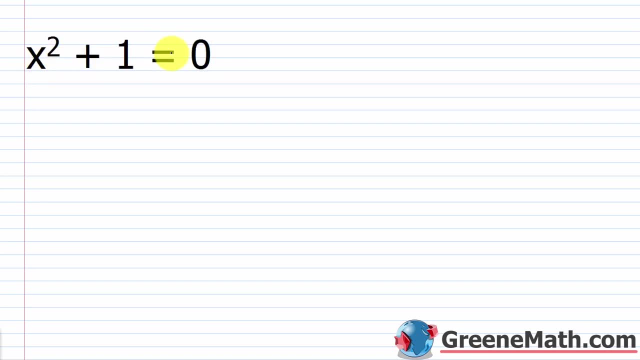 run into this problem. If you see x squared plus one equals zero, let's just start by subtracting one away from each side of the equation, So that would cancel and we would have: x squared is equal to negative one. Now what value can you think of that? you could plug in for x. 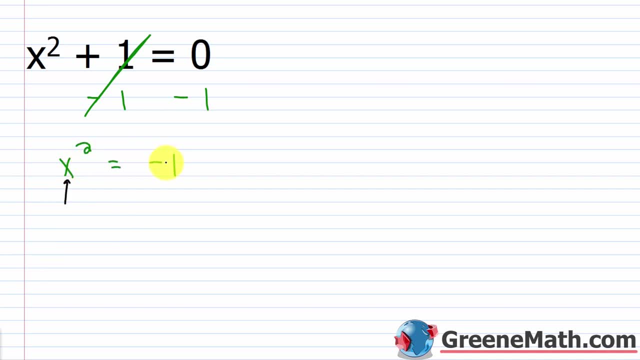 that, when it's squared, would produce a negative one. You can't Again. if I have a real number and I square it, the result is either going to be zero or it's going to be positive. So using real numbers I cannot get a solution. So up to this point we just stop and say there's no. 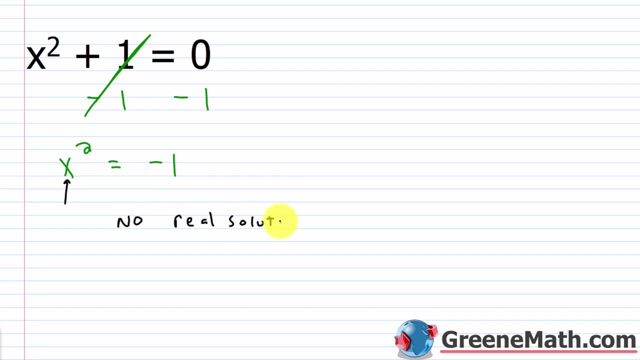 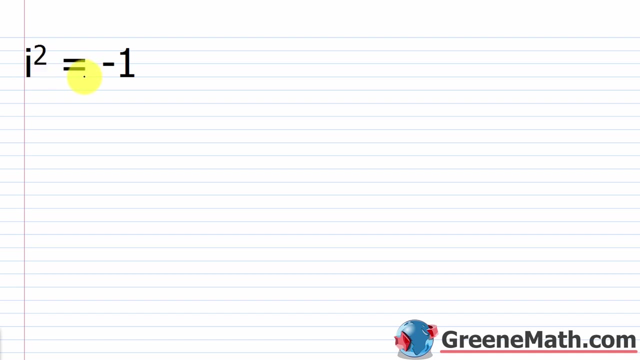 real solution, But in mathematics we always find ways around things. okay. So we're going to introduce today the imaginary unit known as i, and the definition I'm going to give you here is that i squared is equal to negative one. Now, if we were to manipulate this, let's say: we have this, i squared. 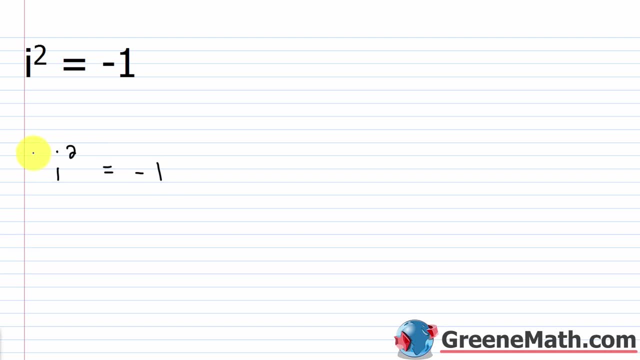 and this equals negative one. If we take the square root of this side and the square root of this side, what's going to happen is this would cancel out the real number system, So we're going to cancel with this and we'll just have i, and this is equal to the square root of negative one. 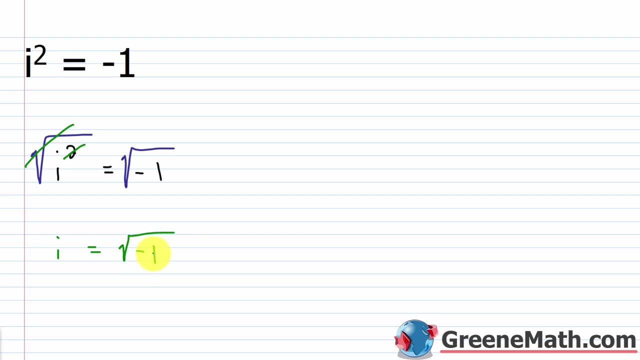 So we can now use this property, this definition, to proceed when we want to take the square root of a negative value. So let's look at an example of this. Let's say: you see the square root of negative nine, And again a lot of students get confused because they're 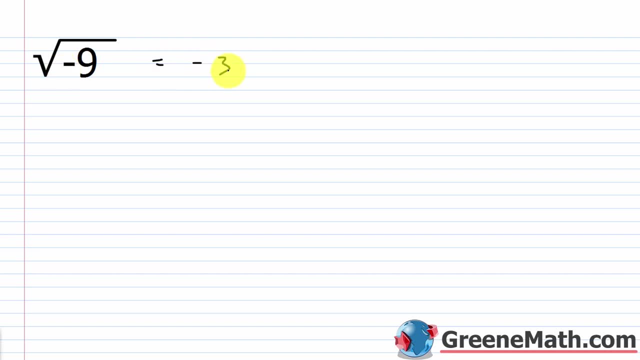 like: oh, I already know how to do that. That's equal to negative three. No, it's not okay. Don't get confused between the negative square root of nine and the square root of negative nine. These are different. This is just the negative of the square root of nine. This is just negative. 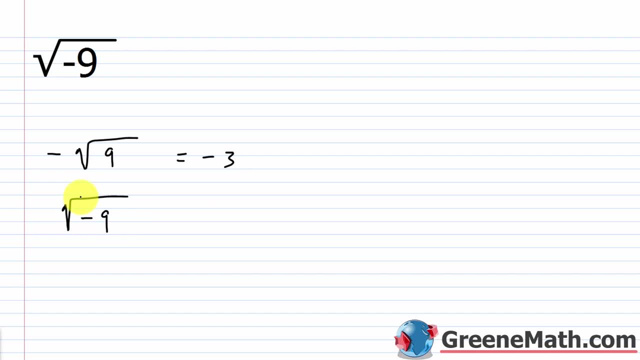 three, With this guy right here, I'm taking the square root of a negative number. This has no real solution. But again, if we define i to be equal to the square root of negative one, we can use a little trick. We can say: this is equal to the square root of negative one. 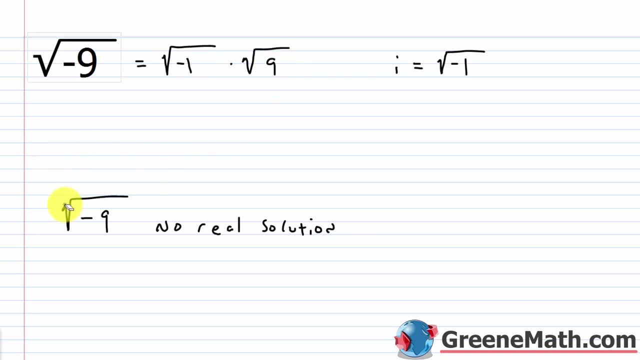 times the square root of nine. Let me erase this real quick. We can replace this right here with i, because i is defined to be the square root of negative one. So I'm going to write that out in front. I'm going to put i out in front: times the square root of nine. 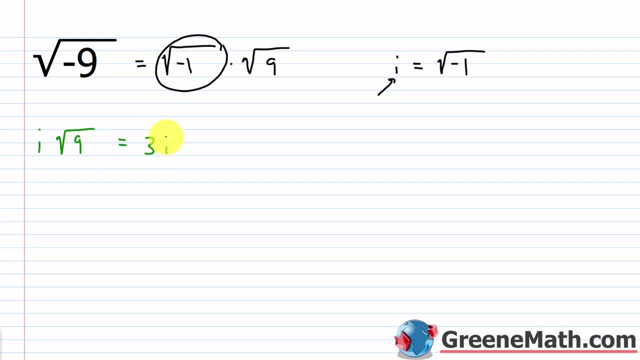 And the square root of nine is just three. So this is three times i, or three i. That's all we're doing. So we found a workaround for this problem of taking the square root of a negative number. Now some people will write this as the square root of nine times. i like that. The reason: 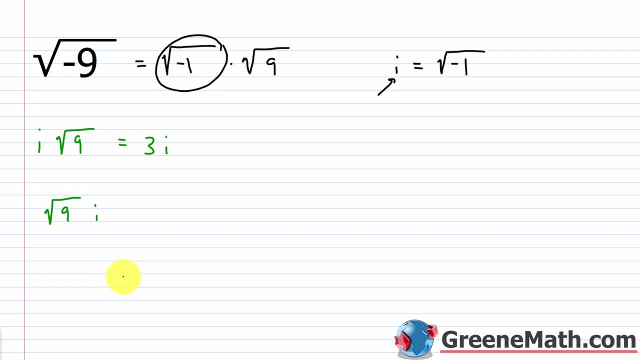 that I don't do that and the reason that most textbooks don't do that is: you don't want to make a mistake. Maybe this is extended a little too far and you think the i is under the square root symbol. You don't want to run into that. You don't want to make that. 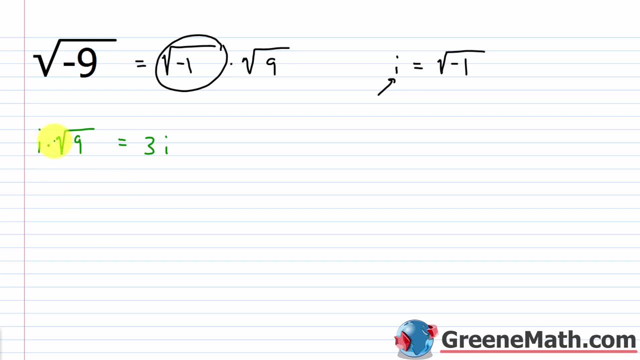 mistake. So to make it crystal clear that i is multiplying the square root of nine, we usually stick it out in front. All right, let's just look at a few practice problems, just to get our feet wet here. So let's suppose you see the square root of negative 10.. So what we're going to do is we're going. 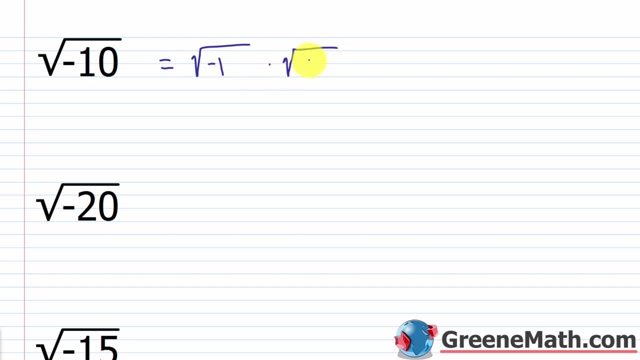 to break this up into the square root of negative one times the square root of 10.. And again, we know the square root of negative one, by definition, is i, So just replace it with i and then times the square root of 10.. The square root of 10,. you can't do anything else. 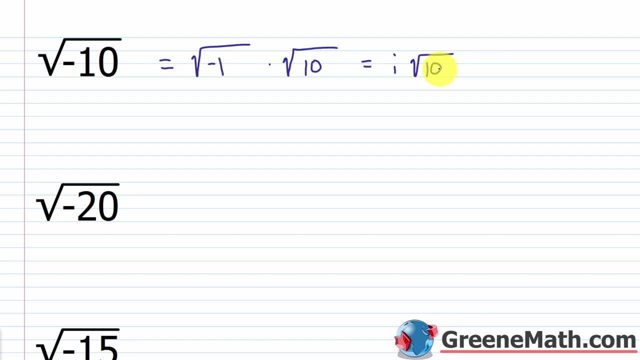 with that, 10 is two times five. No perfect squares there, So we just leave this as i times the square root of 10.. Then we have the square root of negative 20. If you see the negative, you can just go ahead and replace it with an i out in front times. what would 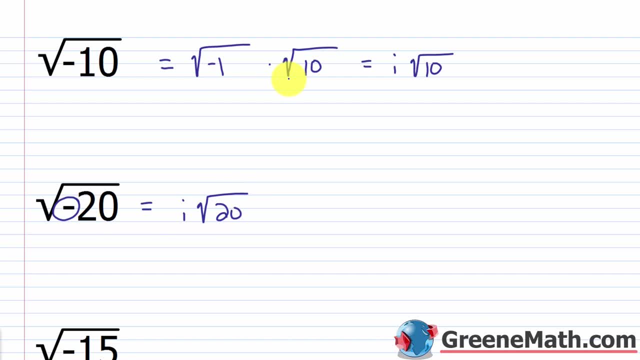 be left would be the square root of 20.. Okay, you don't need to go through this every time, But just for the sake of completeness, let's just keep doing it. So we'll put the square root of negative one times the square root of 20.. So, again, this is by definition. i times. 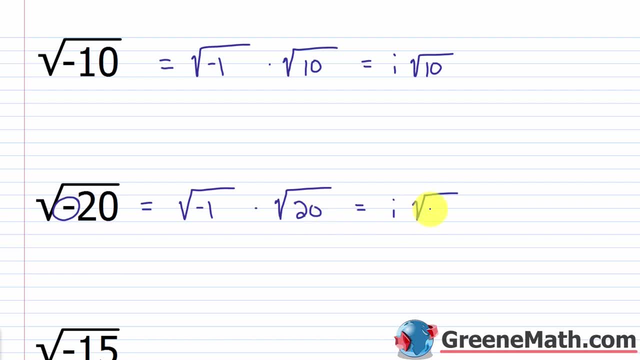 the square root of 20 is what It's four times five. Four is a perfect square. So we're going to do the square root of negative one times the square root of 20, times the square root of five. We know the square root of four is two. So if we completely simplify this, we'll 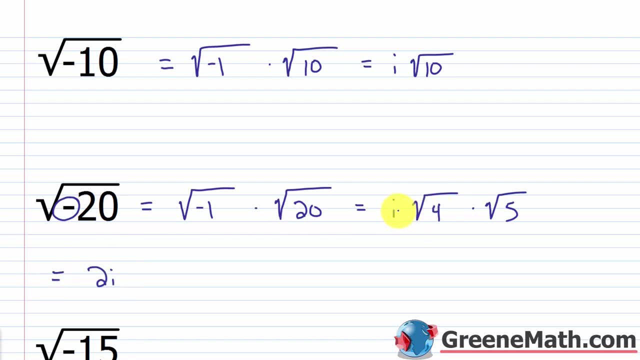 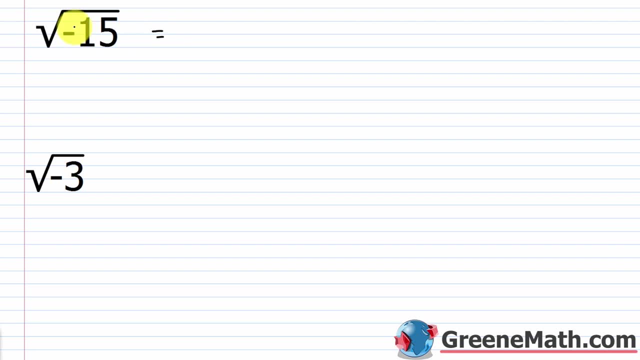 have two i, because again the square root of four is two. two times i is two. i then times the square root of five. For the next one, we have the square root of negative 15.. Again, the shortcut is just to take this: say hey, this is i, and then times the square. 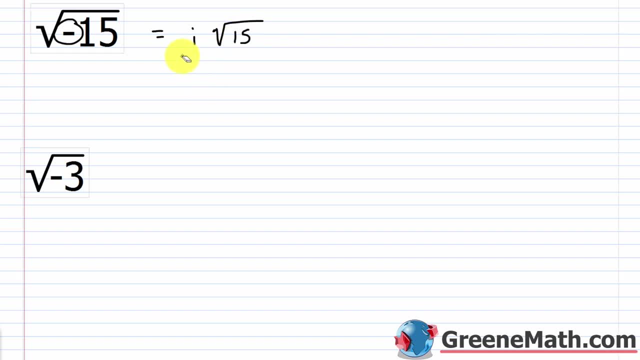 root of 15, and you'd be done, But the long way again. if you just want to realize what's going on here, this is the square root of negative one times the square root of 15.. The square root of negative one is by definition. i then times the square root of 15.. And what? 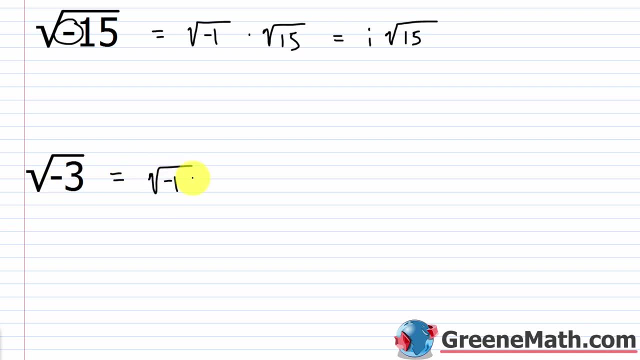 about the square root of negative three. Again, this is the square root of negative one times the square root of three. This is i by definition. so this is i times the square root of three. All right, now we have the negative of the square root of negative 50.. So be very, very. 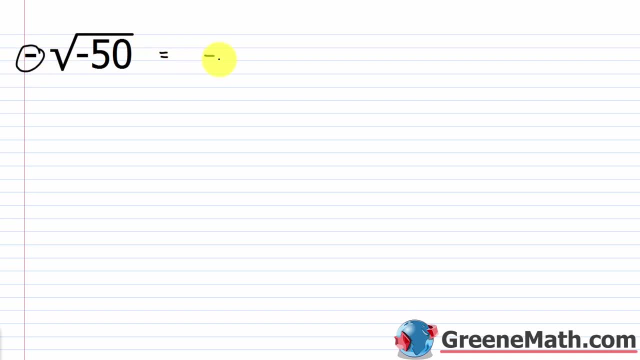 careful here. You have a negative out in front, so let's leave that out in front. Then I'm going to break this up into the square root of negative 15.. The square root of negative one times the square root of 50- we know is 25 times two. 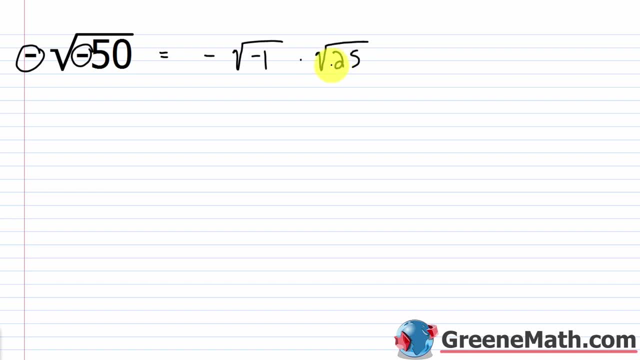 Twenty-five is a perfect square, so let's break that up. We'll put 25 under our square root symbol, then times the square root of two, And we know this has a value of five, so let's just go ahead and replace it. We know this is basically i, So you would have. 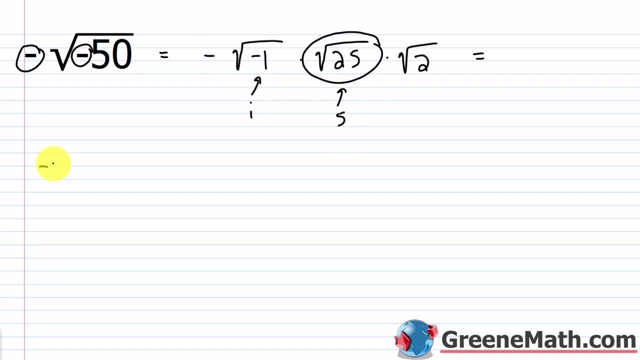 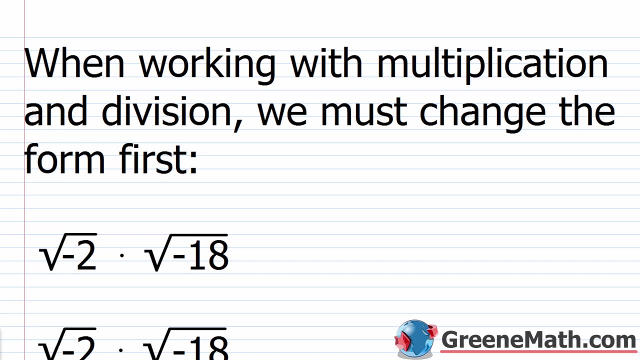 negative i times five or negative five i and then times the square root of two. All right, Let's talk about some kind of immediate applications of this. We want to make sure that you're crystal clear on the product rule for radicals. So when working with multiplication and division, 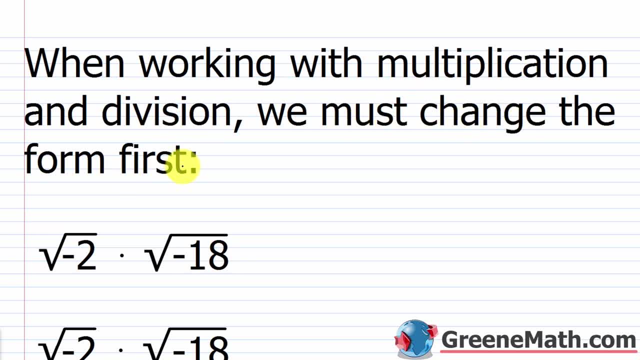 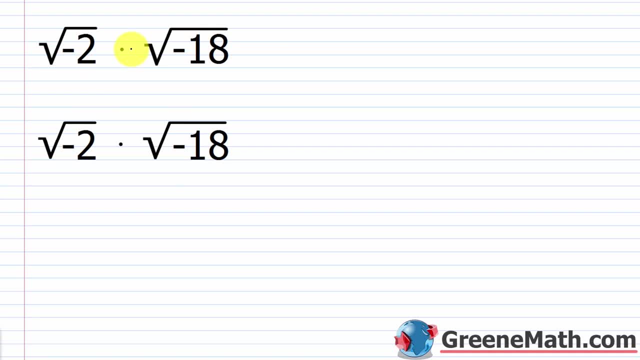 we must change the form first. So here's what I mean by that. Once people know that they're allowed to take the square root of a negative number, the first thing you start seeing on your tests when you give this out, you'll see somebody go: okay, square root of negative. two times square root of negative 18.. That's going to be the square root of negative one. All right, So we're going to go ahead and break this up into the square root of negative two. All right, So we're going to go ahead and break this up into the square root of negative one. 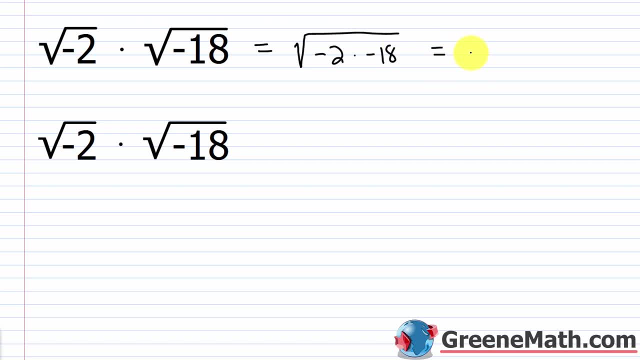 All right, So we're going to go ahead and break this up into the square root of negative one. All right, So we're going to go ahead and break this up into the square root of negative two times negative 18.. This is the square root of 36, which equals six. No, that is wrong. This is wrong, Okay. The correct way to do this problem is to break it up section by section. This right here again becomes i, This right here becomes i. So if we break it up and say we have i times the square root of two. 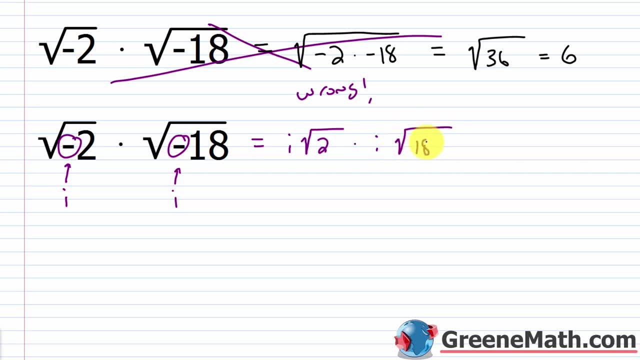 multiplied by i times the square root of 18, what do we get? Well, i times i. by definition is i squared, which is negative one. So let's just put i squared for now. Then times, you'll have the square root of what. Let's break this down. You'll have two times 18 is two times three times three. So essentially, we know that one two would come out and one three would come out. Two times three is six. So what you'd end up with is a square root. 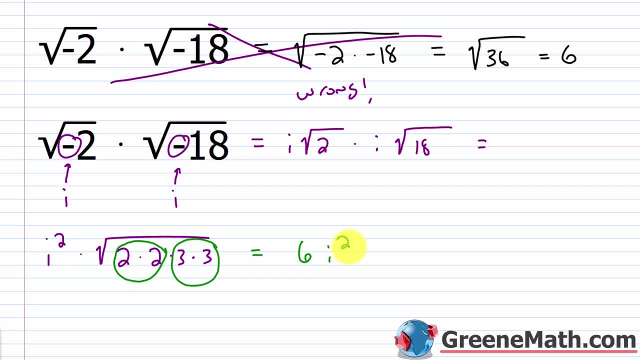 up with is 6 times i squared, and i squared again, by definition is negative 1.. So this would be 6 times negative 1, which equals negative 6.. Now again, if you did this the wrong way, your sign would be incorrect. If you did this like this, you'd end up with positive 6.. That's again not. 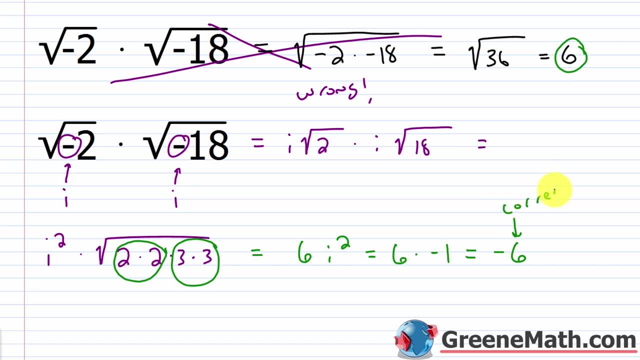 correct. This is the correct way to do it, and then this is incorrect. Okay, this is, this is wrong, So you've got to make sure that you change the form first. Don't just go through and apply the product rule for radicals as you know it, because that's not going to work when you're taking the 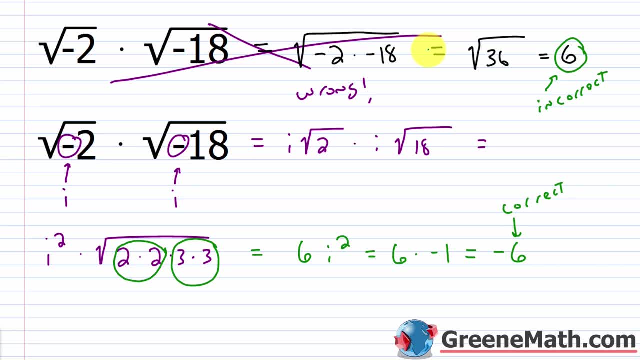 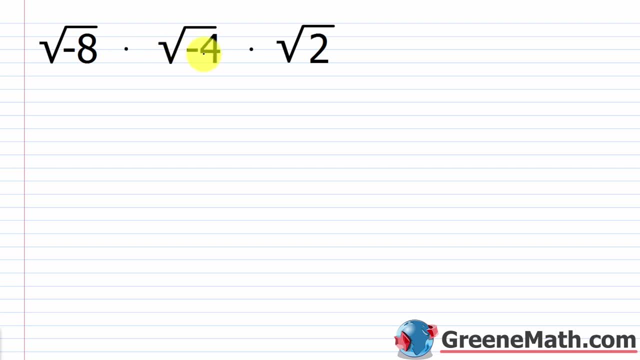 square root of a negative. The same thing is going to apply when we get to a division problem as well. All right, let's take a look at some examples. So we have the square root of negative 8 times the square root of negative, 4 times the square root of negative, 4 times the square root of negative: 4. 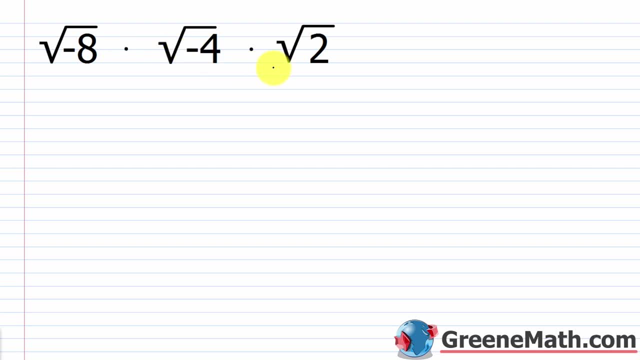 times the square root of 2.. So I can't just say, hey, I have the square root of negative 8 times negative, 4 times 2.. It wouldn't work out that way. What I've got to do is change the form first. 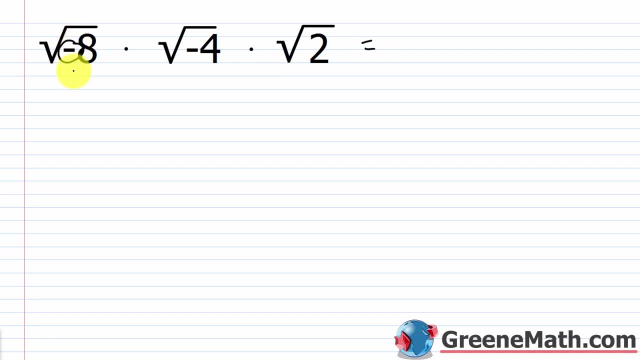 before I do my multiplication. So we all know if we see a negative, we can just replace that with i. We can just replace that with i. So what we do is we say we have i times the square root of 8 would be what It would be the square root of 4 times the square root of 2.. Then you'd have times you've. 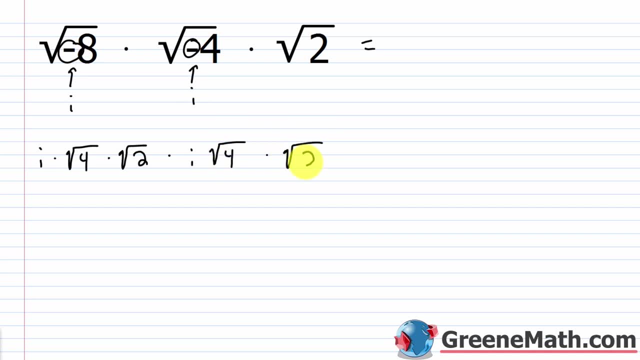 got the square root of 2.. So what is this equal to? Well, we know that this right here has a value of 2.. We know this right here has a value of 2.. And we know, if we took the square root of 2 and 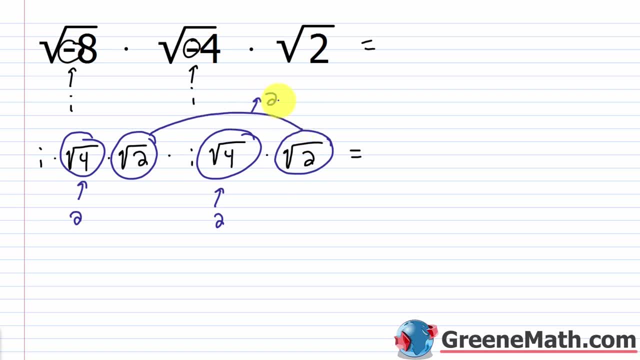 multiplied it by the square root of 2, those two together would have a value of 2.. So what we're going to have is i times i, or i squared, then times 2 times 2, times 2 or 8.. So this ends up being: 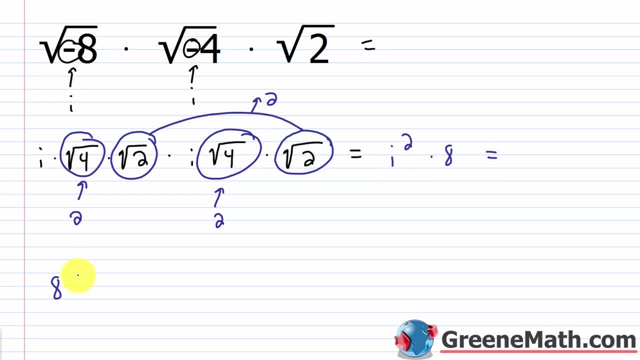 8 times i squared. i squared, by definition, is negative 1.. So 8 times negative 1, which is negative 8.. And again, this is the correct way to do it. If I had gone through and just multiplied and said, hey, this is going to be the square root of negative 8 times negative, 4 times 2, I would 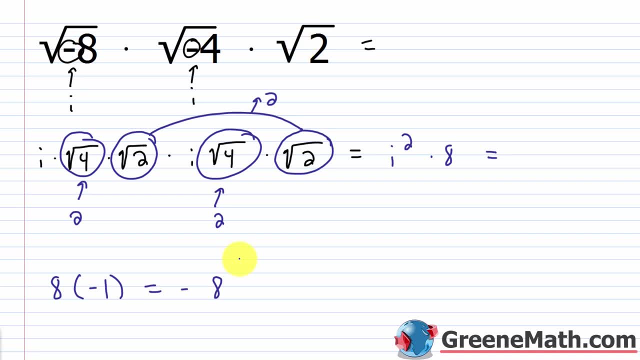 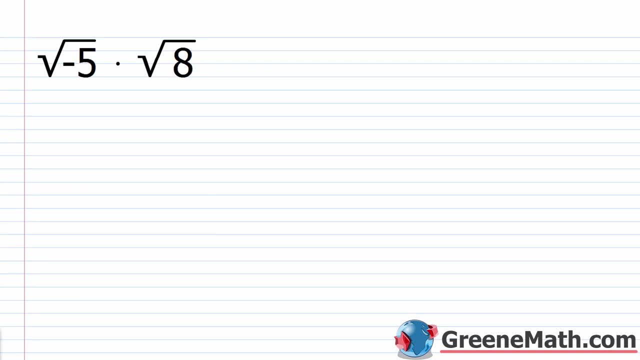 have the square root of 64, which is positive 8.. Right, I would not have ended up with negative 8.. So I would have gotten the wrong answer. All right, what about the square root of negative 5 times the square root of 8?? So again, if I see this, I'll replace. 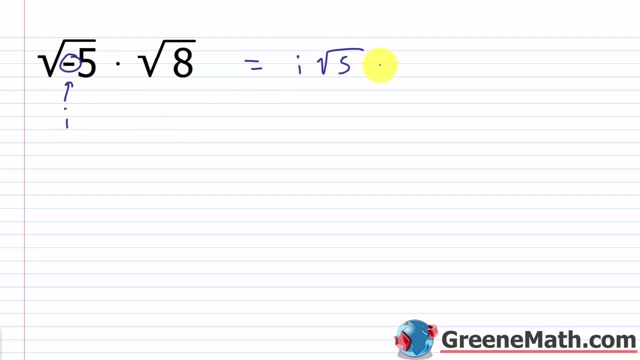 it with i. So this is i times the square root of 5 multiplied by. For the square root of 8, we'll put the square root of 4 times the square root of 2.. So we'll end up with i out in front times the. 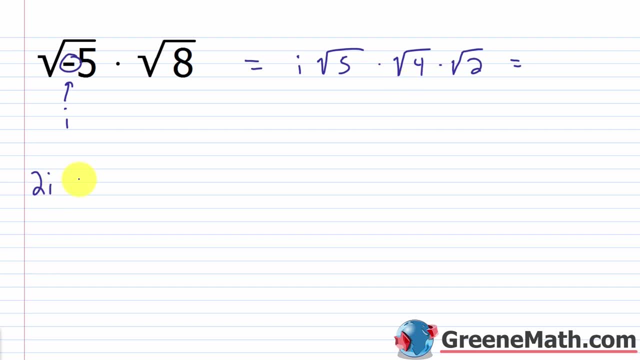 square root of 4 is 2.. So let's put 2i out in front. actually Times the square root of 5 times square root of 2.. Square root of 5 times square root of 2 would be the square root of 10.. So this: 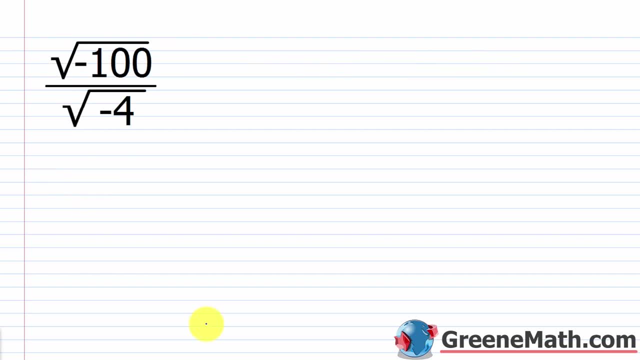 would be 2i times the square root of 10.. All right, now let's take a look at a division problem. So we're going to have a division problem. So I'm going to take the normal variable in f And we're. 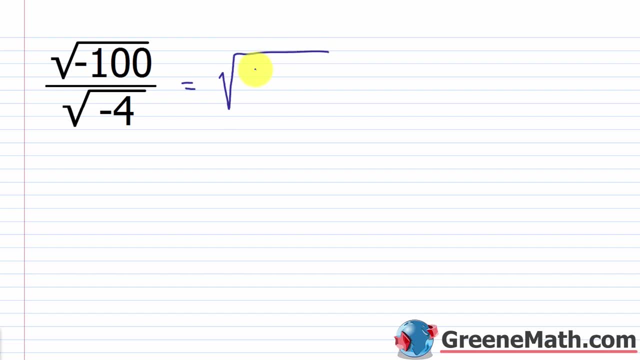 going to use f and i, And I'm going to take the omega i, something like 20, to the power 2.. So here we have the square root of 100 times, the square root of 4 x, the square root of 4 times, or i quote: 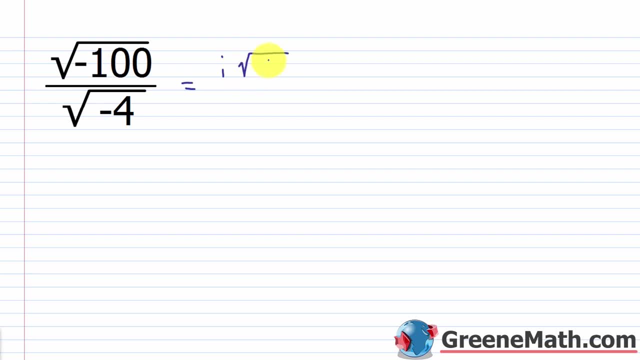 B plus 2i times square root of 4.. By the way, this is the square root of negative 0.. So what I want here is an extension of my integral of negative 1 over the square root of negative 4 times the from. 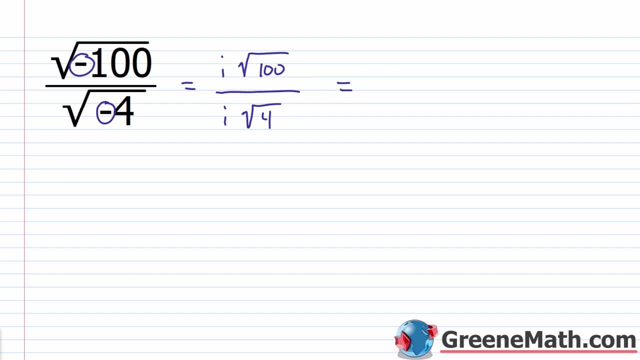 my integral of negative 3.. The sequence you have to do is to line these up fairly for us. here's: how have I over? I Same thing over itself: It's still going to cancel, Still going to cancel. So then you'd have the square root of 100,, which is 10,, over the square root of 4, which. 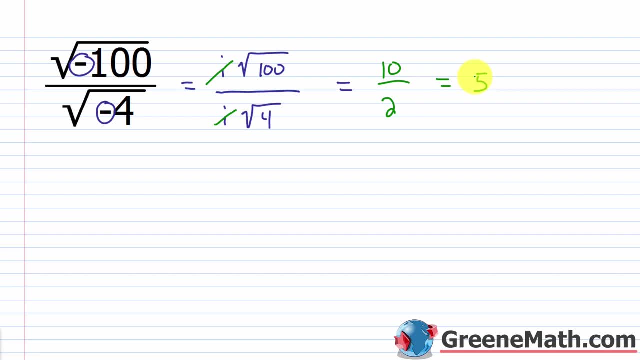 is 2.. Then 10 over 2 is going to give you 5.. Now what about the square root of 28 over the square root of negative 7?? So for this guy right here, what are we going to see? The square root of 28,. we'll write it as the square root of 4 times the square root of. 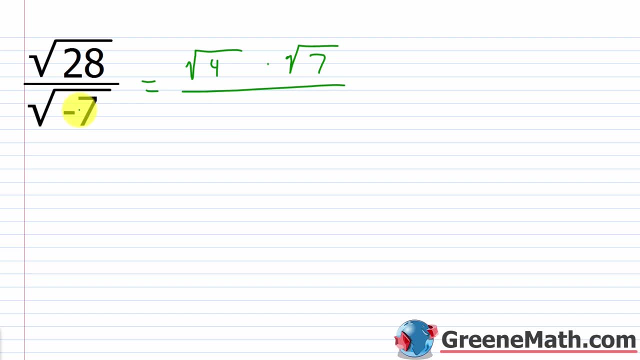 7.. Then for this guy right here, we have the square root of negative 7.. So let's take this out. We'll have I times the square root of 7.. So we know that this would cancel with this, and we know the square root of 4 is just 2.. So this would be 2 over I. Now a lot. 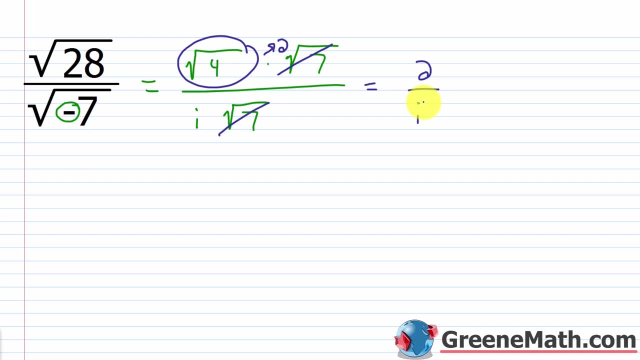 of people will just stop and say, hey, that's my answer. But remember I has a definition of what I is equal to the square root of negative. 1. We do not allow radicals in the denominator Subtitles by the Amaraorg community. 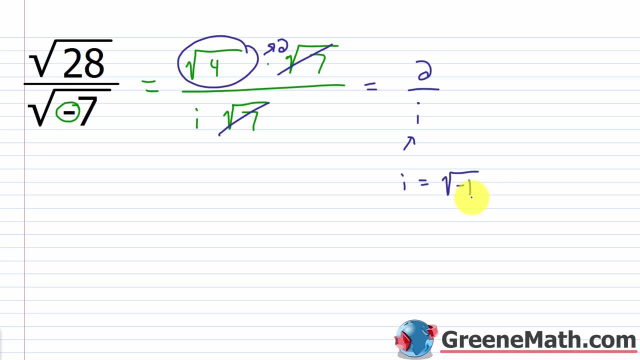 So don't report an answer with I in the denominator, because you're reporting an answer with the square root of negative 1 in the denominator. So what you want to do, you want to rationalize the denominator. So 2 over I. we can just say we'll multiply by I over I. What happens? 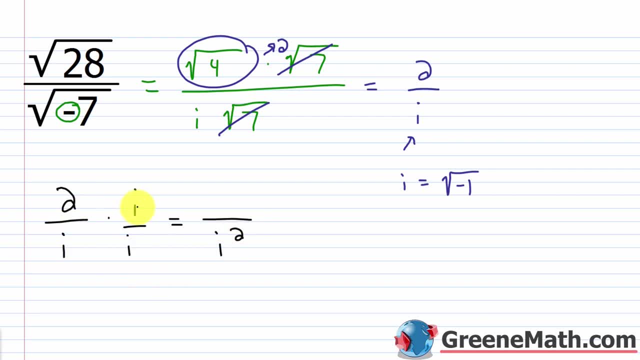 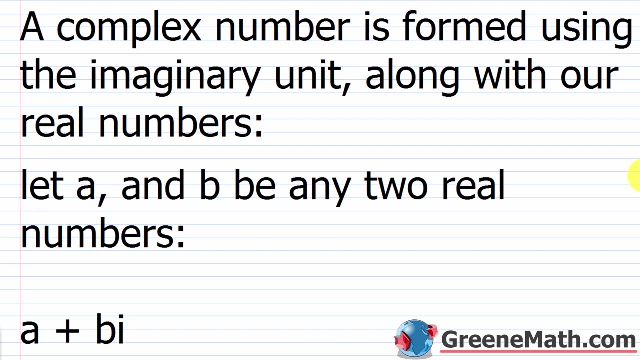 is I times I, is I squared? Then you have 2 times I in the numerator. I squared has a negative 1.. So you get 2I over negative 1, or negative 2I as your answer. All right, so let's talk a little bit about something known as a complex number. So we're 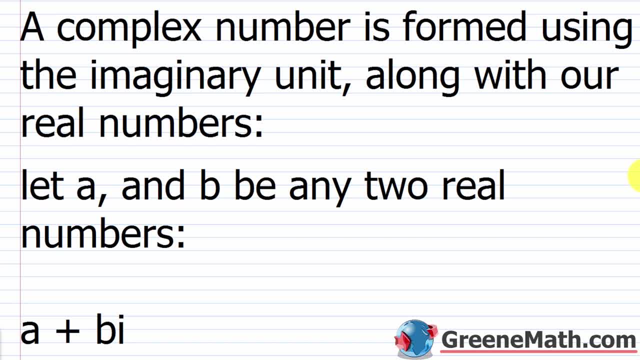 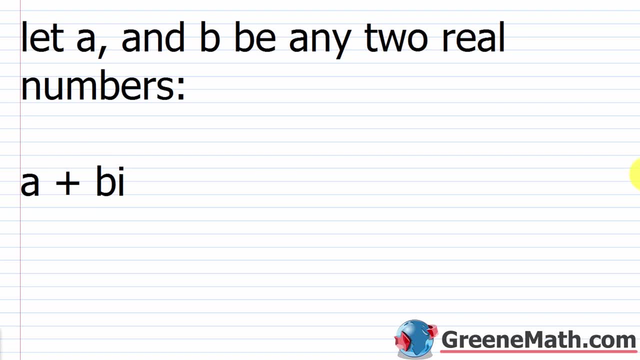 used to just the real number system. Now we're going beyond that. We're talking about the complex number system. So a complex number is formed using the imaginary unit I, along with our real numbers. So you'll generally see this in your textbook written, just this. 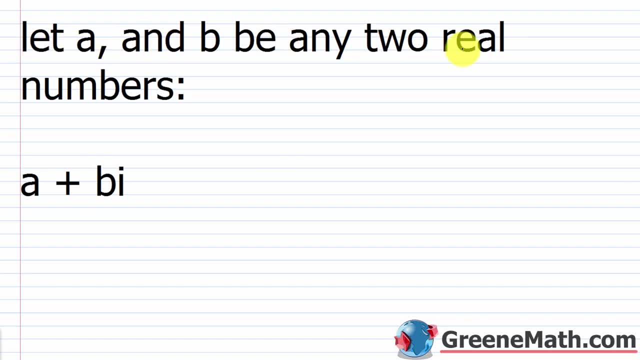 way They say: let A and B be any two real numbers And we'll see our complex number. So this is known as a complex number And it's written as A, which is a real number, plus B, another real number, times I, the imaginary unit. So A is referred to as the real part. 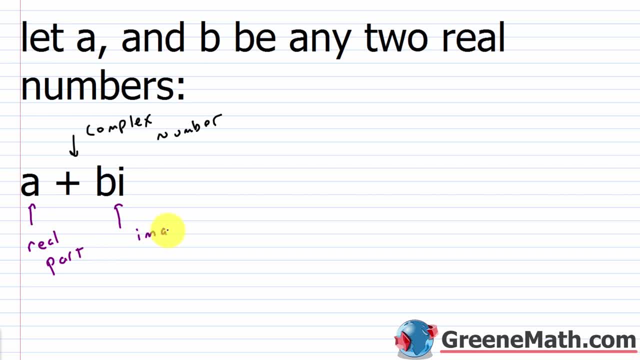 And then B I is referred to. B is referred to as the imaginary part. In some textbooks you will see that only B is described as the imaginary part. Your textbook might say that The textbook I'm using actually says that B I is the imaginary part. It's basically irrelevant. It's not something you 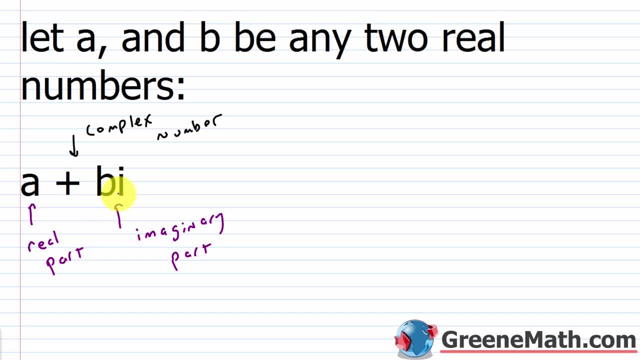 want to argue over. You just need to understand the structure of this so that, when we start working with complex numbers, we know, hey, this is how we can add or subtract them, And we're going to this part right now. So, in order to add or subtract complex numbers, 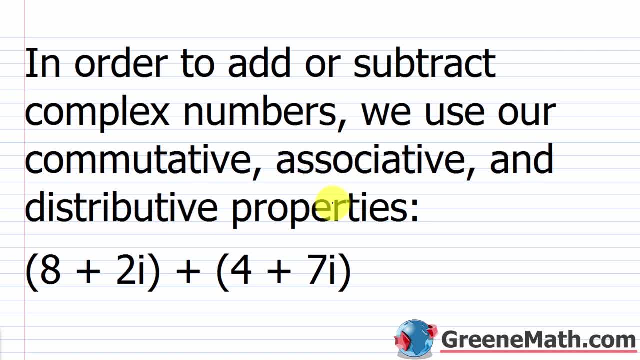 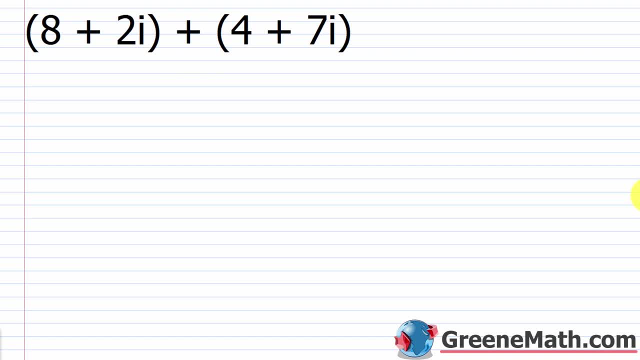 we use our commutative, associative and distributive properties. So we kind of think about this the same way that we think about adding like terms. So if I have something like 8 plus 2x and then I add 4 plus 7x, we all know what to do. We take 8 and 4 and add those. 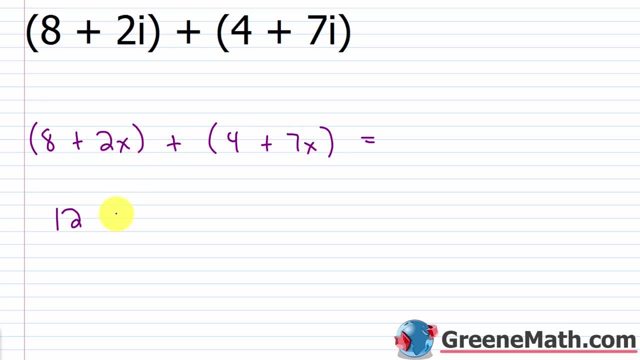 together, That's 12.. And we take 2x and 7x, we'd add those together, That's 9x. Very, very clear what to do. It's the same thing here, okay, So I have 8 plus 4.. So let's group that together: 8 plus 4.. 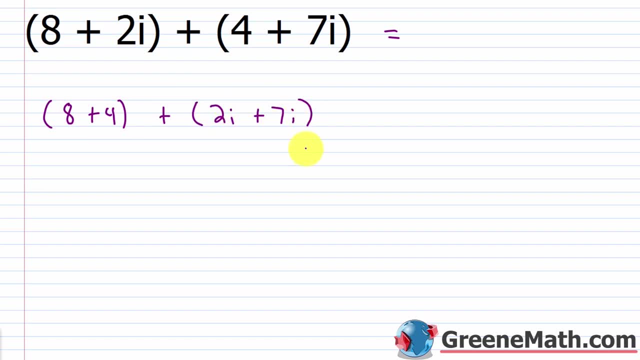 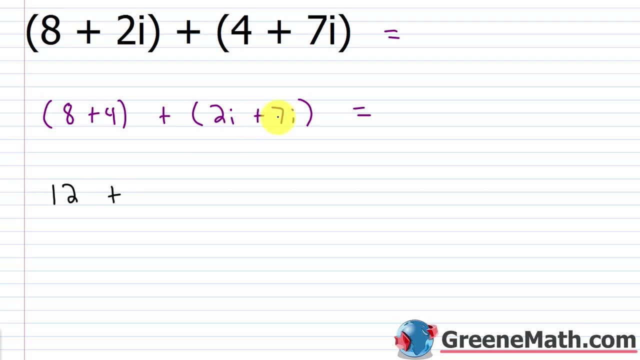 We add 8 and 4.. That's 12.. And then for this guy, 2i plus 7i would be 9i. To make that crystal clear, you could factor out the. i right That's common to each one there, And so you have i times the. 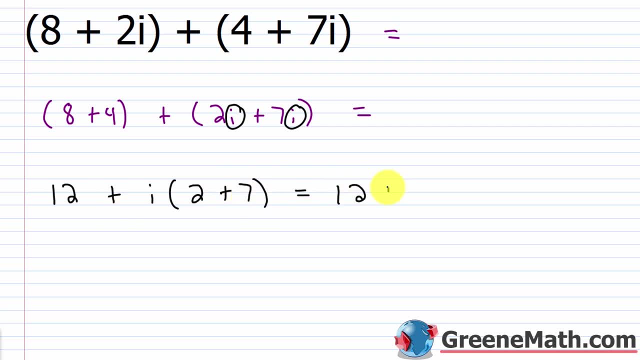 quantity 2 plus 7.. And so this would be: 12 plus 2 plus 7 is 9, times that i there, So you end up with 12 plus 9i. So it's just like adding like terms. It's the same principle. 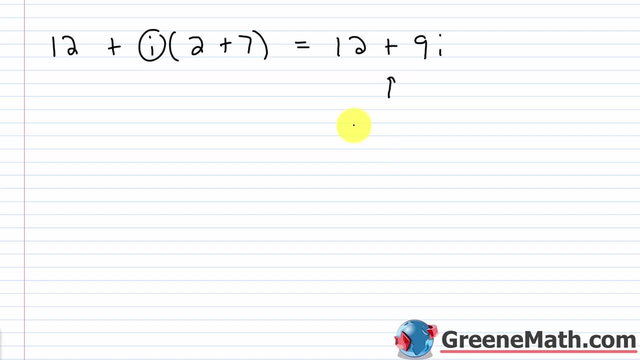 here Now, when we see it like this, where we have a- the real i, the real, i- the real i, the real part, plus bi- the imaginary part. this is known as standard form for a complex number. So when you write something, you want to write it that way. You don't want to put 9i plus. 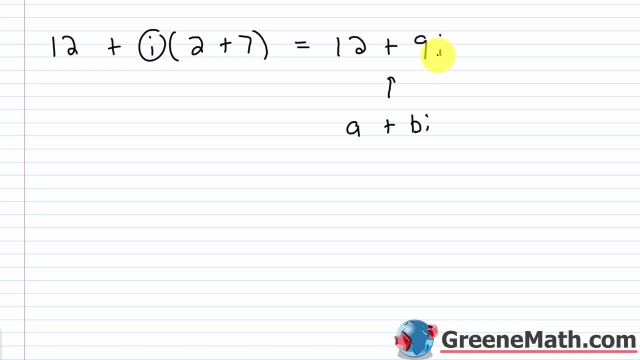 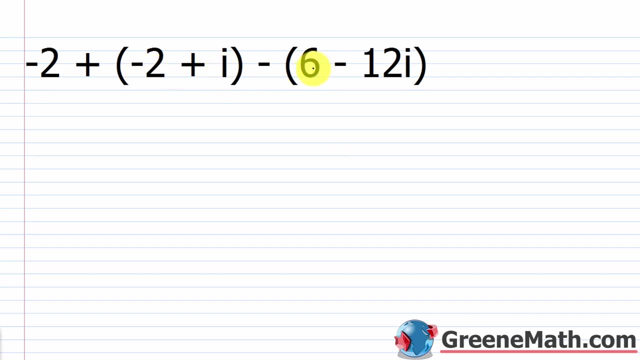 12. You want to put 12 plus 9i. Well, let's take a look at another one. We have negative 2 plus we have negative 2 plus i, minus the quantity 6 minus 12i. So we have negative 2 and then plus negative 2 plus 9i. 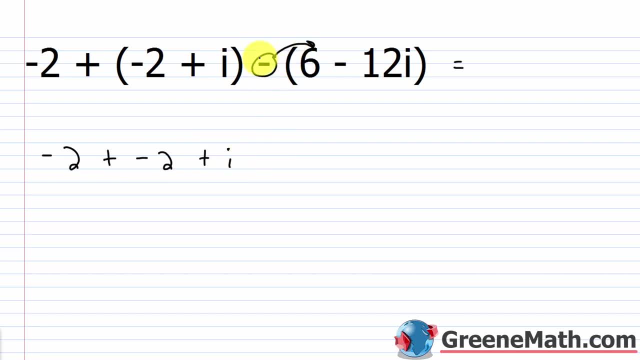 This will again get distributed to each term, So you'll have minus 6, and then minus a negative 12i would be plus 12i. So negative 2 plus negative 2 is negative 4.. Then negative 4 plus negative 6 is negative 10. And then we have i plus 12i, which is 13i, And again. 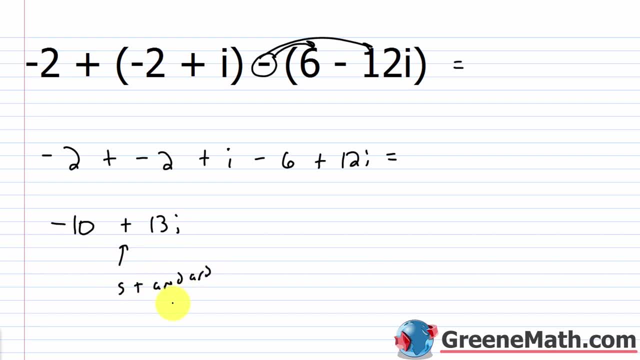 we wrote this in standard form. This is a plus bi, Your real part plus your imaginary part. Let's take a look at one more of these. We have 7 plus 4i plus negative, 8 plus 8i plus 2 minus 2i. So again, if I just go through and say, okay, the real parts, 7 plus negative. 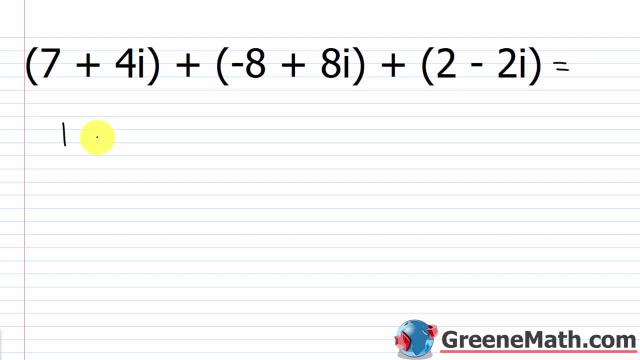 8 is negative: 1. Negative 1 plus 2 is positive, 1. Then your imaginary parts. you've got 4i plus 8i minus 2i. So 4 plus 8 is 12.. 12 minus 2 is 10.. So this is plus 10i. 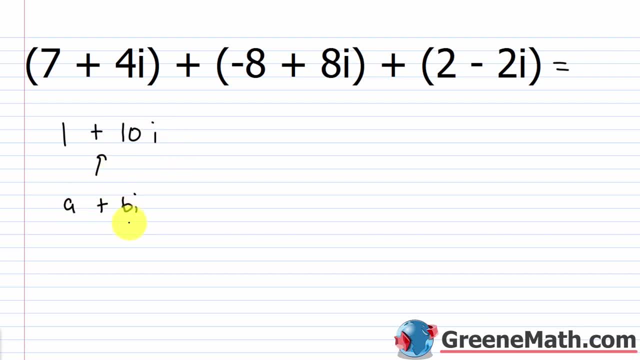 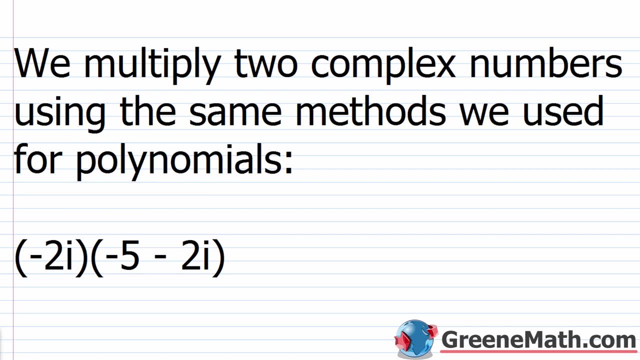 And again, this matches the a plus bi. This is your standard form. All right, now let's talk about multiplying two complex numbers together. We basically use the same methods we would use for polynomials. So if we had a single term, polynomial or a, 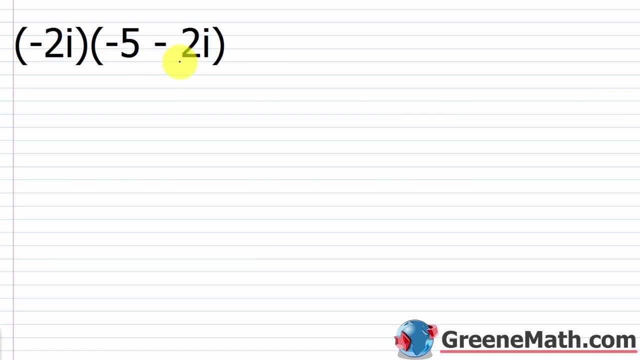 monomial multiplied by a two-term polynomial or a binomial. what would we do? We'd just use our distributive property. You'd have negative 2i times negative, 4i plus 5i plus 2i times negative 5. that'd be positive 10i. and then you'd have negative 2i times negative 2i. 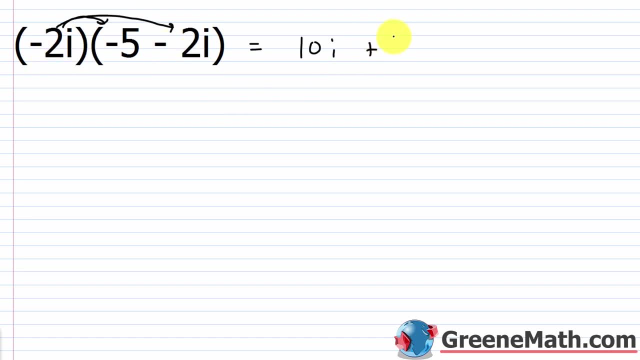 that would be positive. 2 times 2 is 4. i times i is i squared. now, i squared has a definition of negative 1, so this is 10i plus 4 times negative 1, which is basically 10i minus 4. now, this is not. 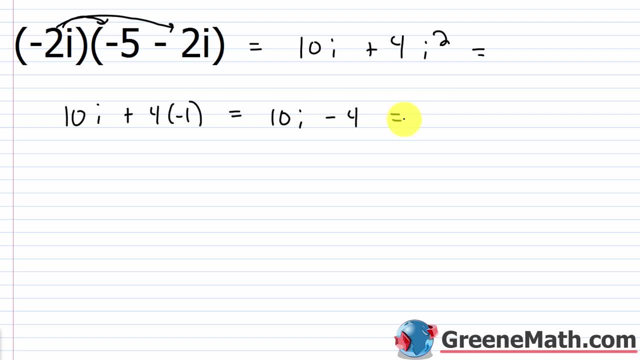 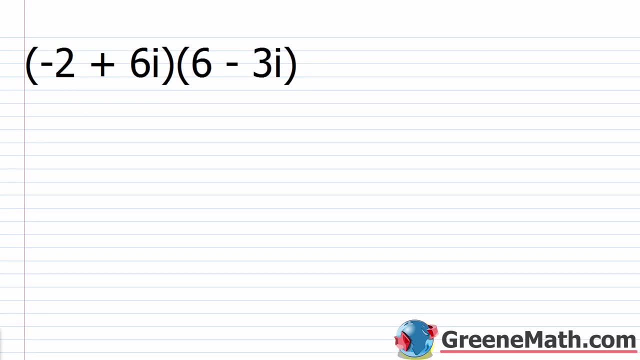 in standard form. you want the real number first, so we're going to switch the order and say this is negative 4 plus 10i. all right, now we have something that looks like the product of two binomials. so for something like this we can use FOIL. we have negative 2 plus 6i. that quantity. 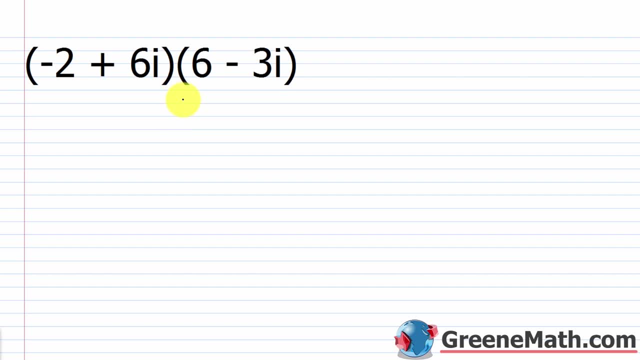 multiplied by the quantity 6 minus 3i. so if i look at the first terms, negative 2 times 6 would be negative 12. if we look at the outer terms, negative 2 times negative 3i would be positive 6i. if we look at the inner terms, 6i times 6 would be positive 36i. and then the last terms: 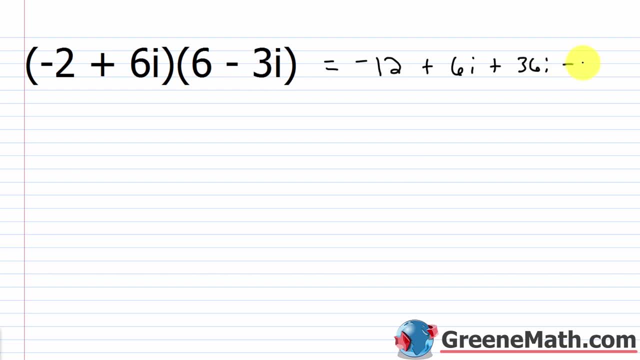 6i times negative 3i would be minus 18i squared, so we have 6i and 36i that could be combined, so we'll have negative 12 again. 6 plus 36 would be 42. so plus 42i and then minus 18i squared. 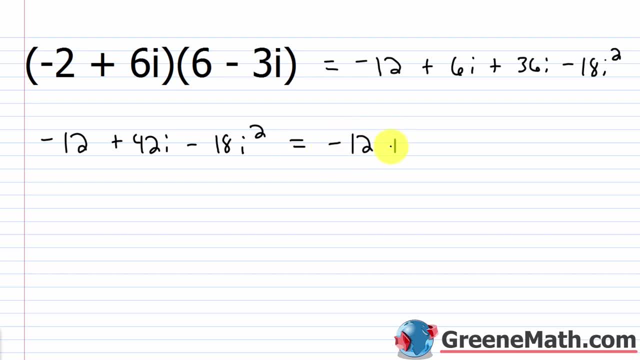 so we're going to look at the inner terms. 6i times 6 would be positive 36i. and then the last- we're not done. We have negative 12 plus 42i. Here's the big thing: i squared is negative. 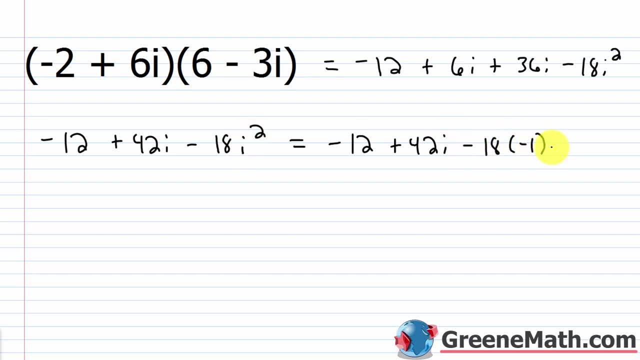 1. So this would be minus 18 times negative 1. So we know that negative 18 times negative 1 is positive 18. So essentially you'd have negative 12 plus 18 plus 42i Negative 12. 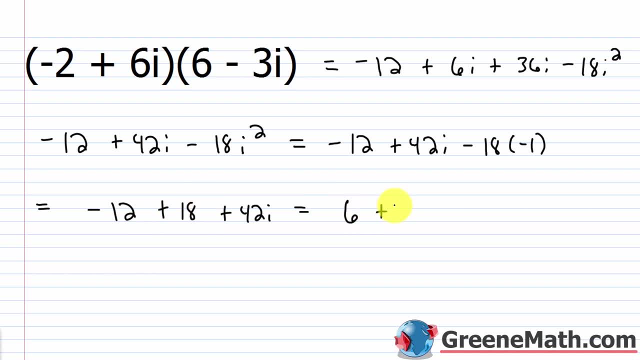 plus 18 is 6.. So we end up with 6 plus 42i. Again, this is in standard form. You've got your real part plus your imaginary part, All right. so let's take a look at one more of these And just like if I was multiplying three binomials together, I would multiply. 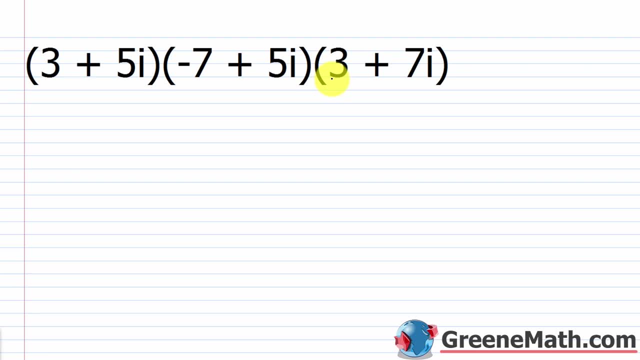 two of them. first find that product, then multiply the result by the third. So we have 3 plus 5i, that quantity multiplied by the quantity negative, 7 plus 5i multiplied by the quantity 3 plus 7i. So let's start by multiplying these two together And what's? 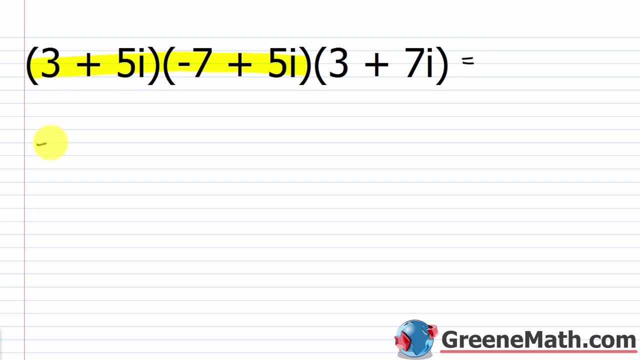 that going to give us. So for FOIL 3, FOIL 3 times negative 7 is negative 21.. The outer 3 times 5i would be positive 15i. The inner 5i times negative 7 will be minus 35i. And then the last 5i times 5i is 25i squared. 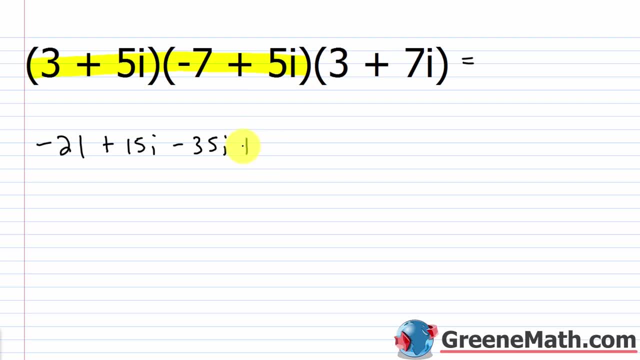 Now we know i squared is negative 1.. So let's just go ahead and write: plus 25 times negative 1.. And again, this is times this guy right here. We'll do that in a second. Let's just simplify first and then we'll multiply by this. 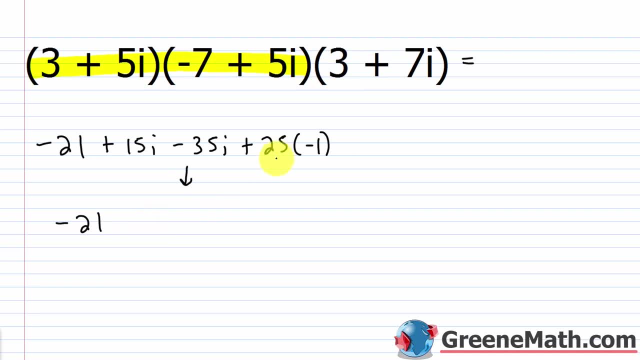 So this would be equal to what You'd have: negative 21.. 25 times negative 1 is negative 25.. So let's put minus 25.. And then 15 minus 35 is negative 20.. So minus 20i, So negative. 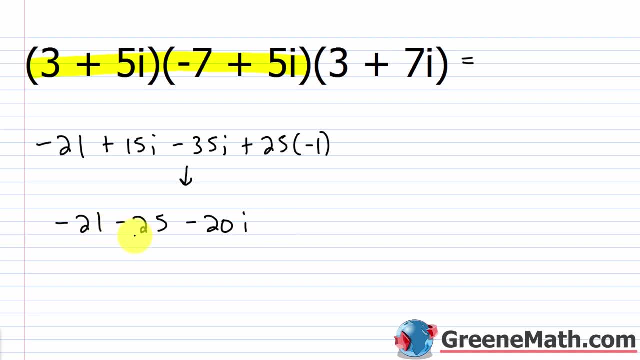 21 minus 25 is negative 46. So let's erase this And we're going to write negative 46, then minus 20i, And this will be multiplied by 3 plus 7i, So we can use FOIL again here. So negative 46 times 3 is going to give us negative 138. 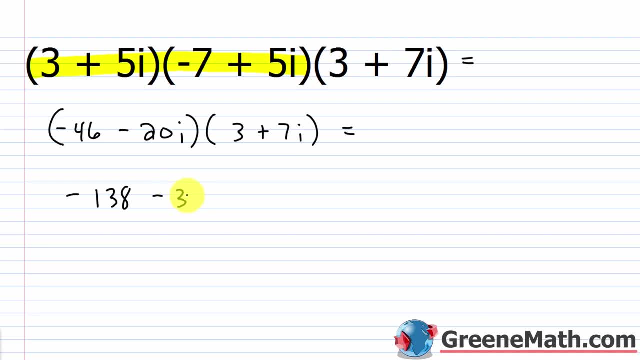 The outer negative 46 times 7i is negative 322i. The inner negative 20i times 3 is going to give us negative 60i, And then the last negative 20i times 7i is going to be negative 140i squared. 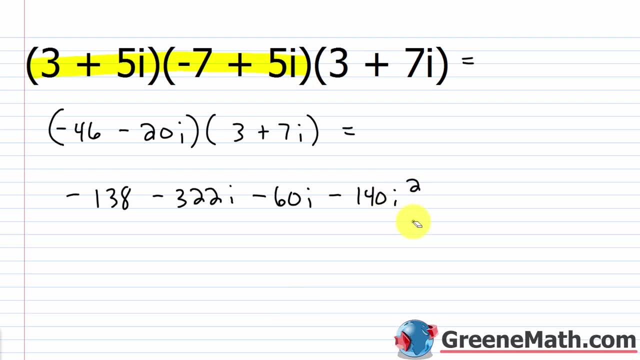 All right Now, remember i squared- is negative 1.. So let's just replace that, Let's just replace this with negative 1.. And so what we'd have is negative 140 times negative 1, which is positive 140.. So positive 140 plus negative 138 would give us 2.. Then negative. 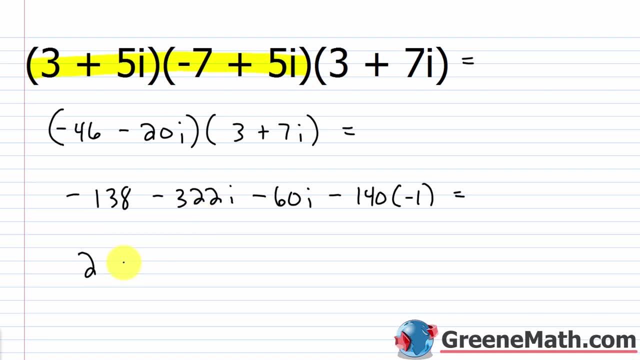 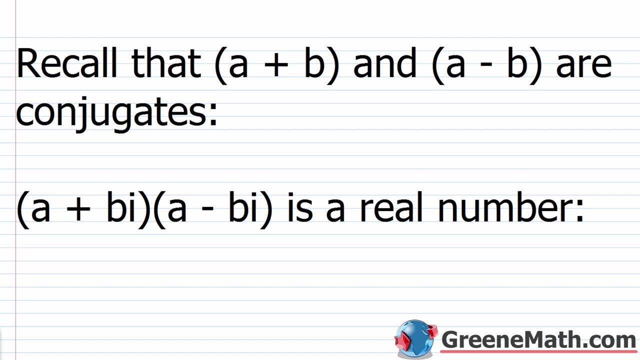 322i minus 60i would be negative 382i. So as our answer in standard form, we have 2 minus 382i. All right, Let's talk about division. Now, when you work with division, you're going to need to think: 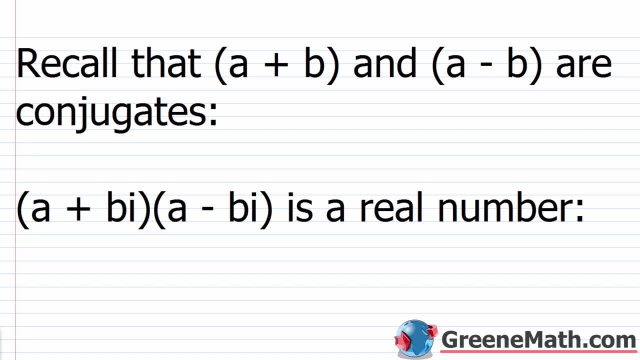 back to when you rationalized a binomial denominator. We did that in a previous lesson, So recall we talked about this thing known as conjugates. So we have a plus b and a minus b. Those are conjugates. If you multiply them together, you use FOIL, You end up with a squared minus. 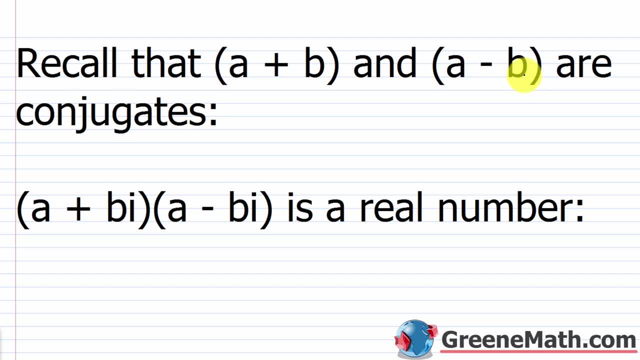 b squared The middle, two terms will drop out. It's not going to be any difference. when you're working with division You're going to need to think back to when you rationalized a binomial denominator. So here you'll have a complex conjugate. So a plus bi times a. 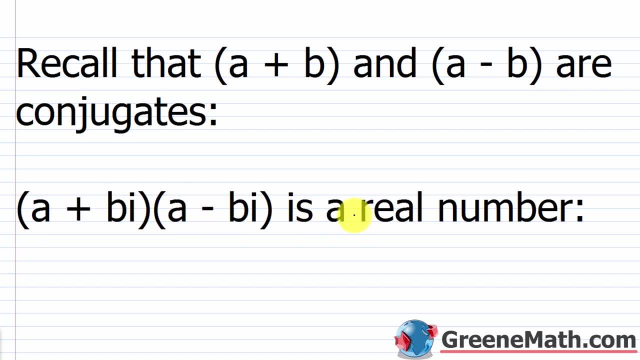 minus bi. Those two are complex conjugates And the result is a real number. Now, normally, if you have a plus b multiplied by a minus b, you get a squared minus b. squared With this, a plus bi, multiplied by a minus bi, you're going to end up with a squared plus. 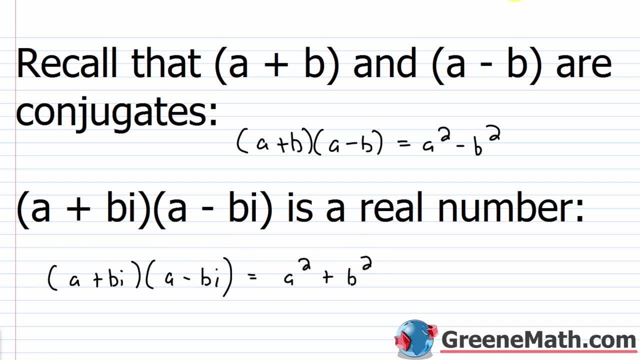 b squared. So you're going to need to think back to when you rationalized a binomial denominator. This is a big source of confusion. Here the sign is negative, Here it's positive. Why do you think that is? It's because of this. i times i, which is i squared, which is a. 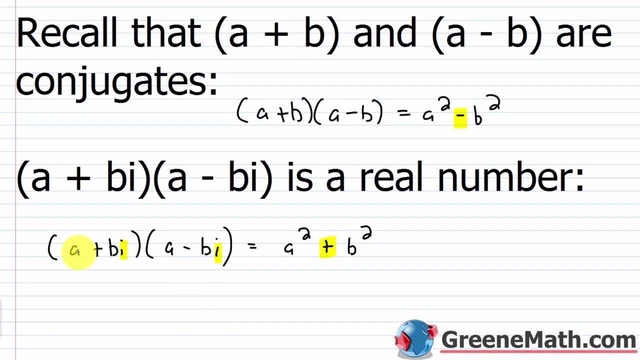 negative 1, which changes the sign. So if we went through and did this, a times a is a squared. The outer a times negative bi is minus abi, The inner bi times a is positive abi And the last bi times negative bi And the last bi times negative bi And the last. 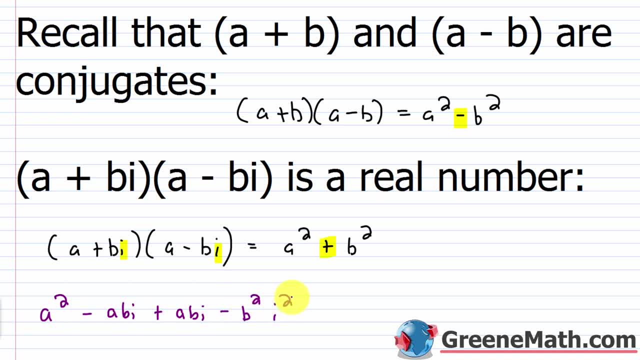 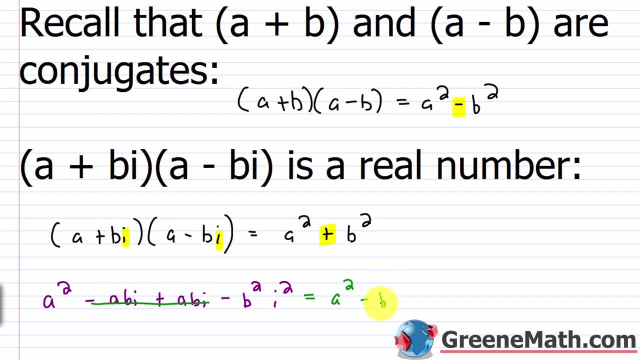 bi times negative. bi is minus b squared i squared. Now we know already that this would cancel. So what do we have? We have a squared minus b squared i squared is negative 1.. So times negative 1. All that's going to do is change the sign If you have a negative. 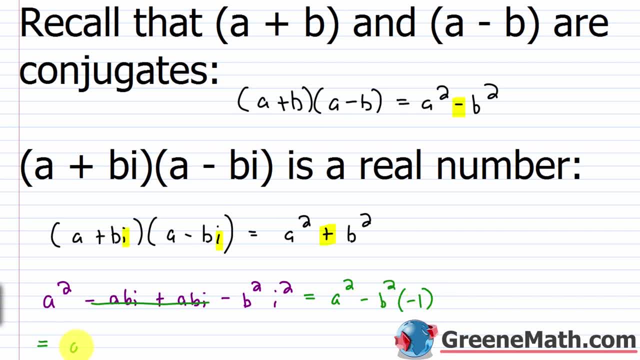 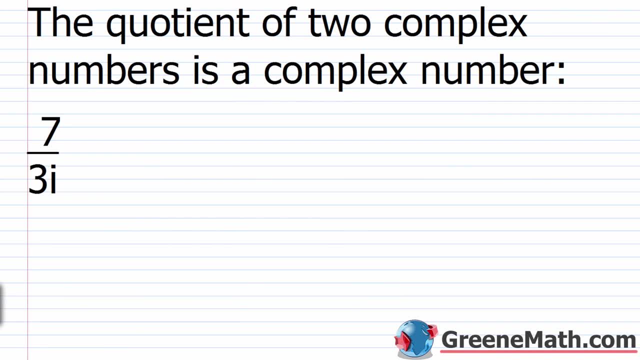 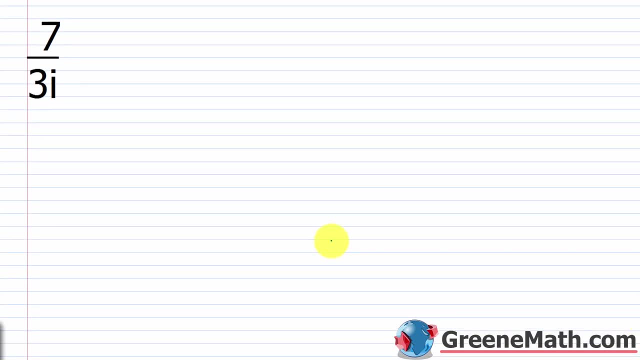 times a negative, you end up with a positive. So this gives me a squared plus b squared. So that's where the difference in the sign comes in. So the quotient of two complex numbers is a complex number If we start out with something simple like 7 over 3i- We already talked about earlier. 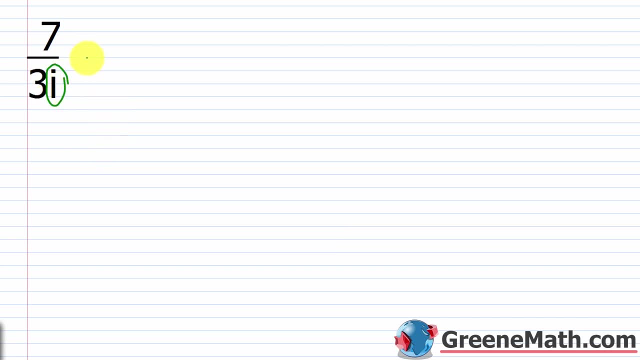 the fact that i is what It's: the square root of negative 1.. So we don't want to leave it like that. We want to multiply by i over i, Basically the same thing we've been doing to not have a radical in the denominator. This is going to give us 7i over 3i squared. 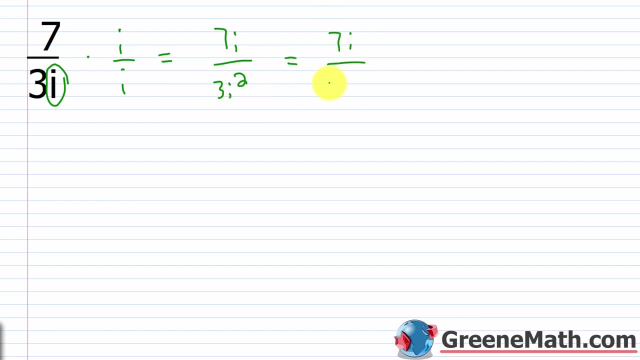 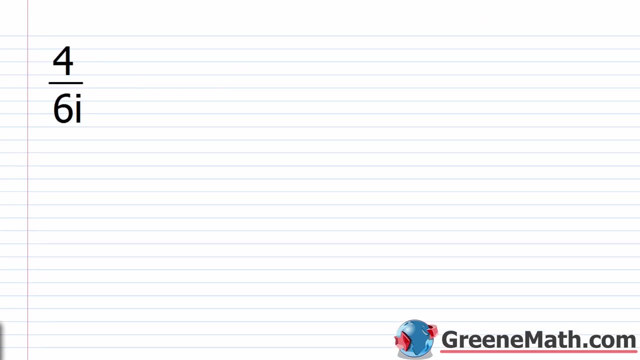 Again i squared- is negative 1.. So this is 7i over negative 3.. And, of course, you could also write this as negative 3i, All right, so what about something like 4 over 6i? Well, the first thing you would do, 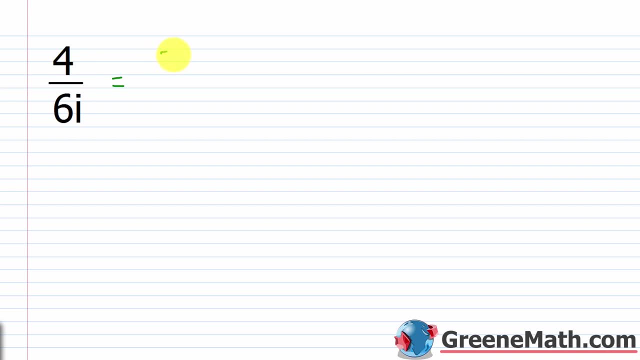 is just reduce. They're each divisible by 2.. So this would be 2 over 3i. And then again, because i represents the square root of negative 1, we just multiply by i over i. We'll end up with 2i over 3i squared. i squared is negative 1.. So we'll end up with what? 2i over negative. 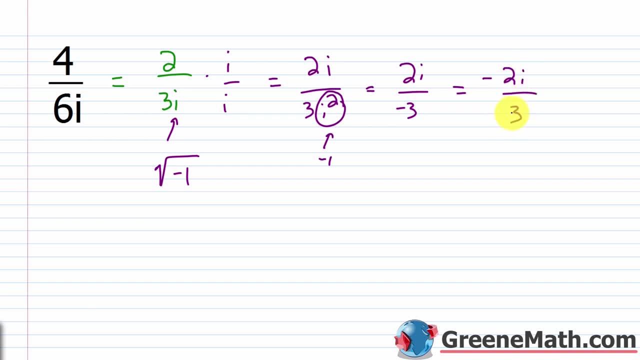 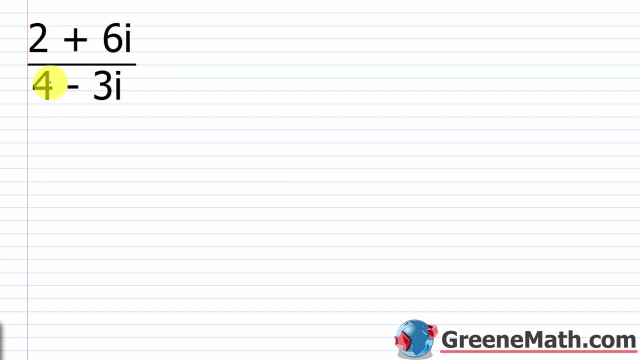 3.. All right, now let's take a look at one where we're going to need to multiply by the complex conjugate, So we have 2 plus 6i over 4 minus 3i. Again, i is the square root of negative. 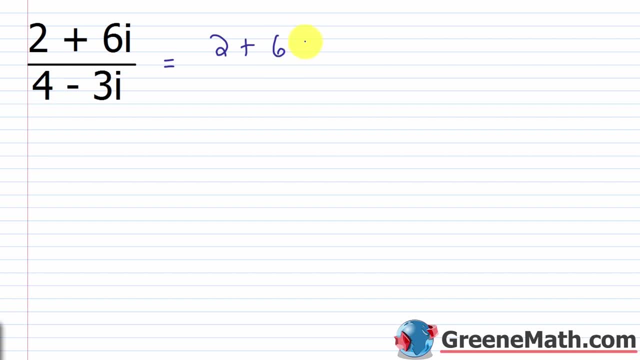 1. So really we could write this as: 2 plus 6 times the square root of negative, 1 over 4 minus 3 times the square root of negative 1.. We don't want radicals in the denominator, so we want to rationalize. 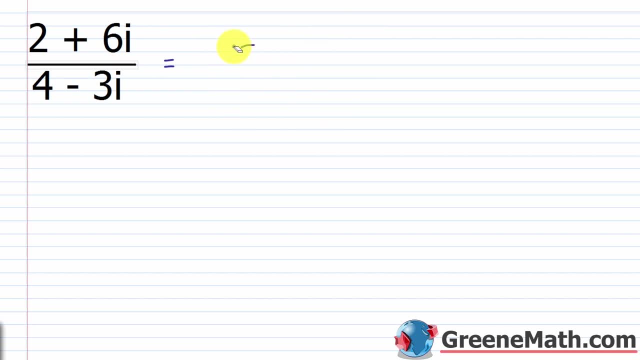 So we want to rationalize, All right. so if we want to do that, what would we do? Again, we worked with binomial denominators before, So we multiply both the numerator and denominator by the conjugate of the denominator. In this case it's going to be no different, So the terms stay the. 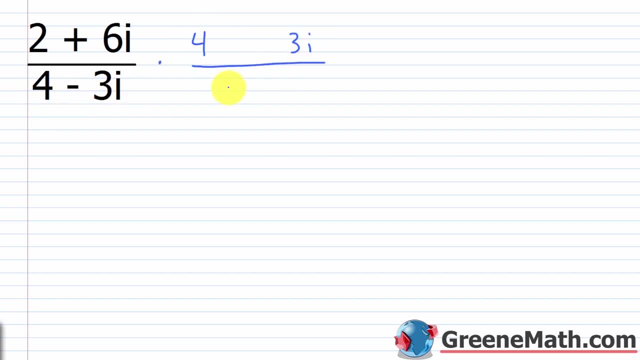 same, 4 would be the same and 3i would be the same. It's just that the sign is going to be different. Here it's a subtraction, so this is going to be addition. Now, in the denominator it's a breeze, because we know the formula. It's a squared plus 6i over 6i. 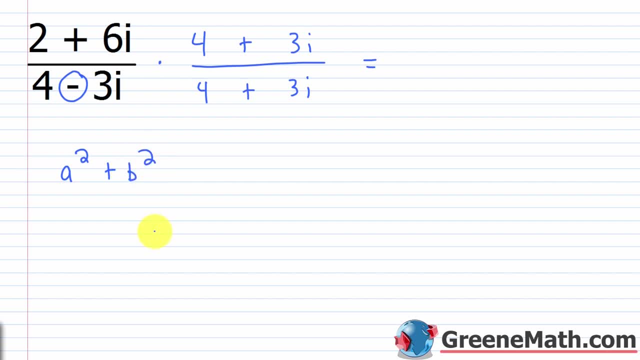 All right. so if we want to do that, what would we do? Again, we worked with binomial denominators plus B squared, And again the reason it's plus is because of that I squared being equal to negative one. it's going to change the sign, So we'll go through this the quick way we'll go. 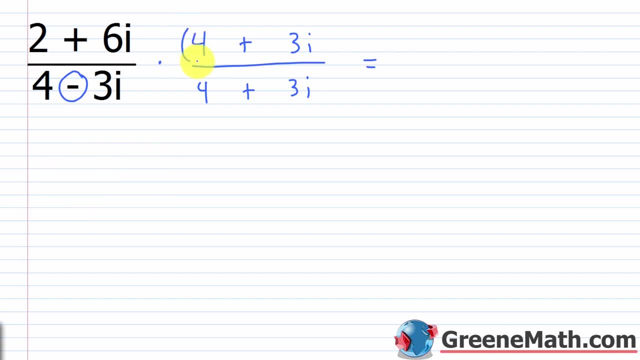 through it the long way, Let's do it the long way first. So if we do FOIL that first two times four is eight, then the outer two times three I is plus six I. the inner six I times four is plus 24 I. 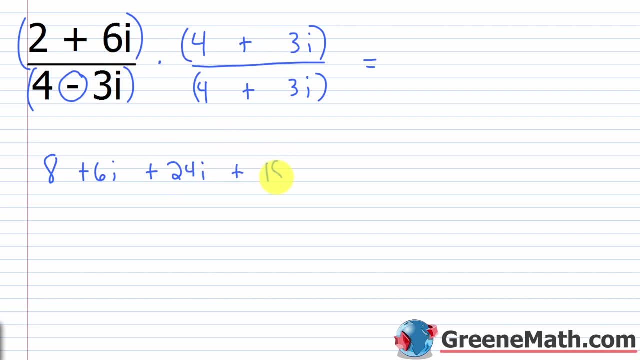 then the last six. I times three, I would be plus 18, I squared. Now we know this has a value of negative one, so we can replace it, But let's just continue for now. In the denominator again, the quick way is to realize that this follows a formula that's A squared, So four squared is 16. 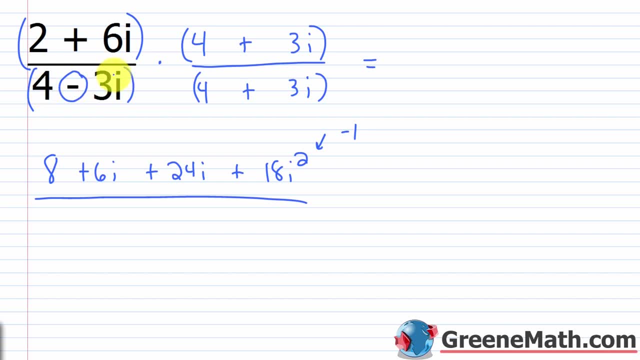 plus B squared. B in this case is three. forget about the I, it's just a three. So three squared is nine. So you'd have 16 plus nine, which is 25.. Now, I'm going to do this the long way. 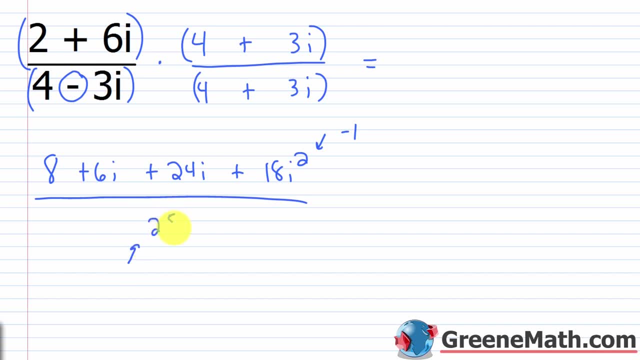 and you're going to see that this denominator down here is going to end up being 25 in the end. So four times four is 16, the outer four times three I is plus 12 I. the inner negative three I times four is minus 12 I. and the last negative three I times three I would be minus nine I. 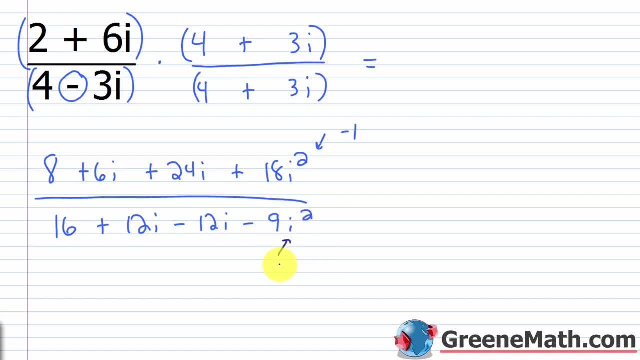 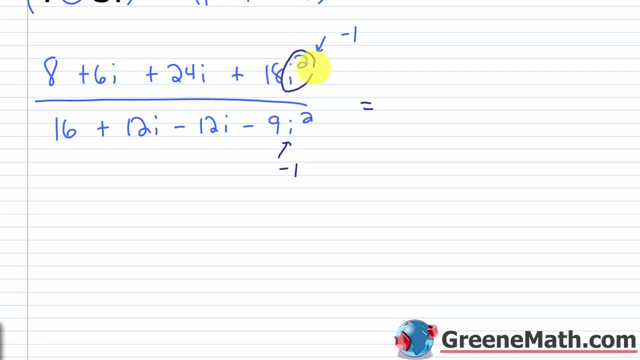 squared Again. this I squared here has a value of negative one, so keep that in mind. So we scroll down, get a little room going. If this I squared is negative one, really, I have 18 times negative one which is negative 18.. Negative 18 plus eight would be. 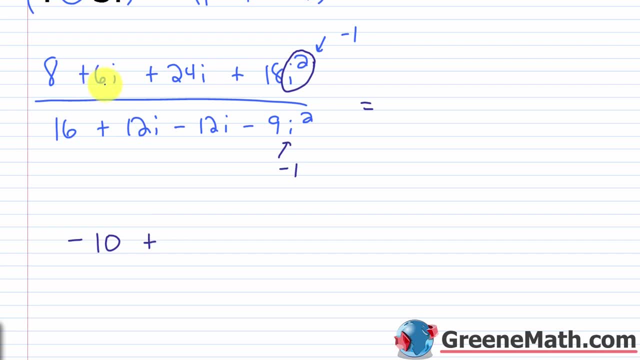 negative 10.. So this is negative 10.. Then, plus six I plus 24 I is 30 I and this is over. You'd have 16 plus 12 I minus 12 I. this is going to cancel And you basically have negative nine times negative. 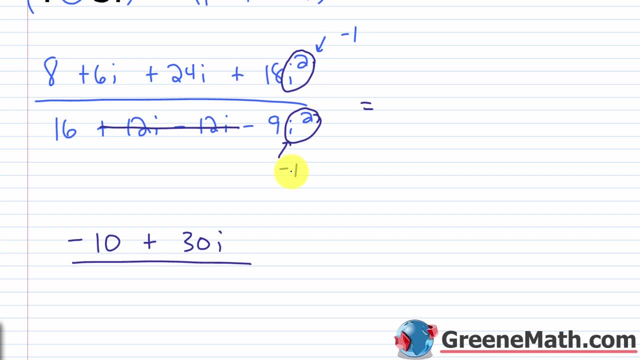 one, because again this is negative. one Negative nine times negative. one is positive nine. So you've got 16 plus nine, which again is 25.. So that's the long way to do it. The short way again: A squared plus B squared, If you just. 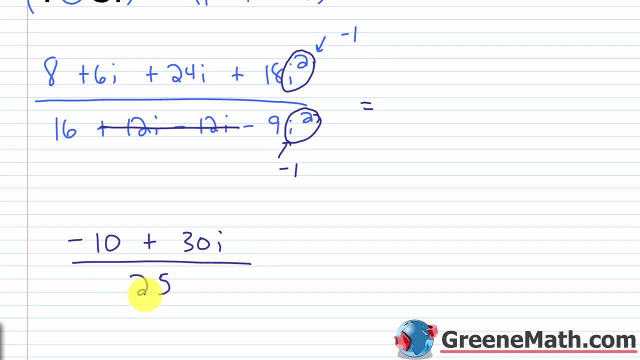 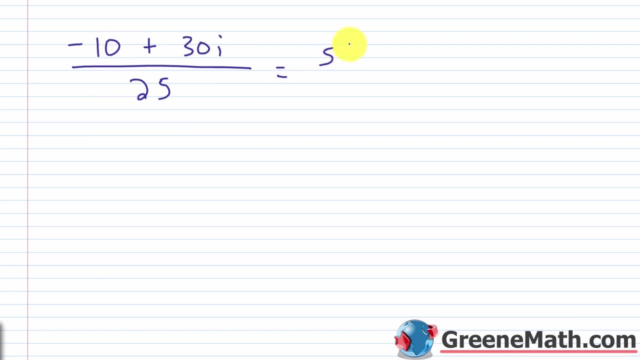 remember that you can calculate that denominator very quickly. Now we're not done, because we can simplify this further. Everything there is divisible by five. So let's factor out a five, We'd have negative two plus six. I, inside the parentheses over, we'll write this as five times. 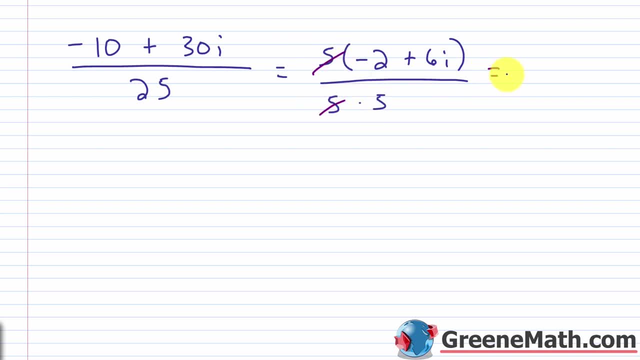 five. We'll cancel a common factor of five between numerator and denominator and we'll report our answer as negative. two plus six, I Over five. Or, if you wanted to, you could say this is negative: two-fifths plus six-fifths. 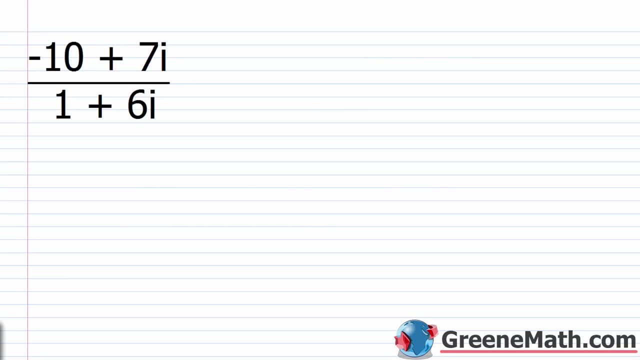 times I. Either answer is acceptable. All right, for the next one, let's use our little shortcut for the denominator. We have negative 10 plus seven, I over one plus six, I. Again. we'll multiply the numerator and denominator by the complex conjugate of the denominator. 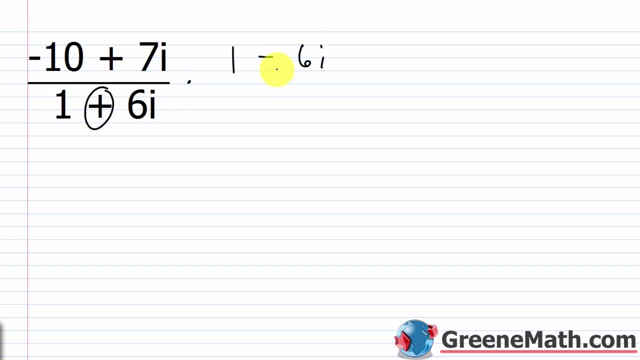 So this would be one instead of plus, it'll be minus and then six. I over one minus six I. 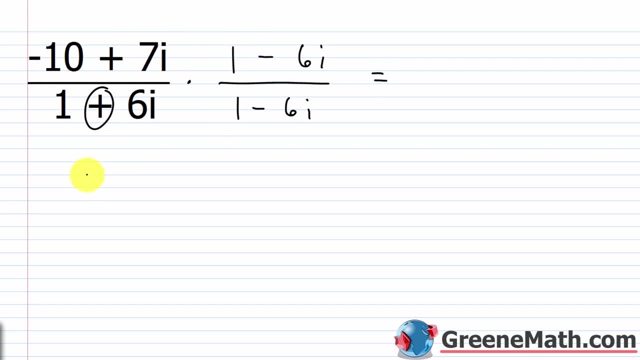 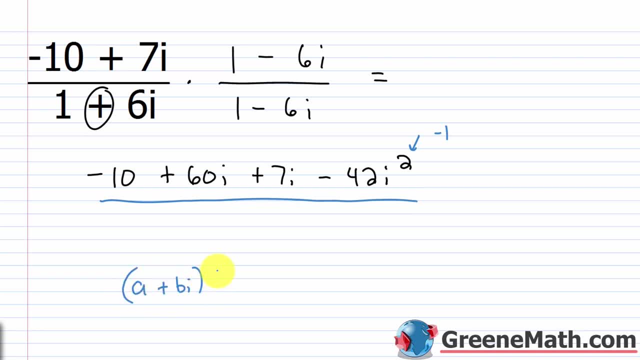 We know that if we have A plus B I, multiplied by A minus B I, this is equal to what It's A squared- okay, the first value squared plus B. okay, not the. I forget about the I B squared. 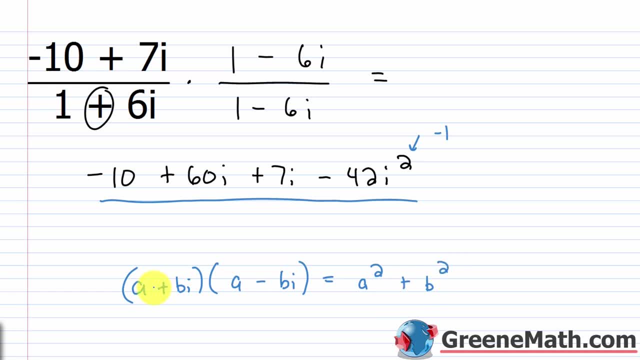 So, following this, I would take 1,, which represents A here, and square it. that's just 1.. Then I would take 6,, which represents B here. forget about the I. that's already calculated for you with the sign. 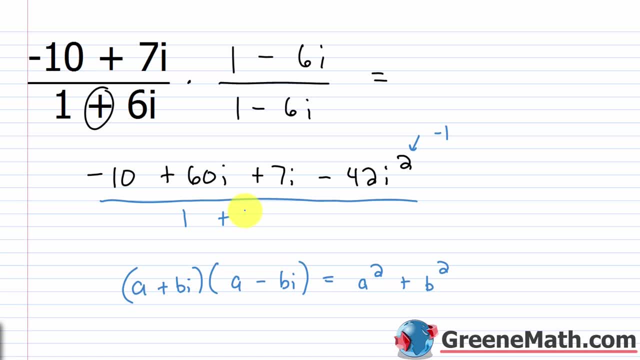 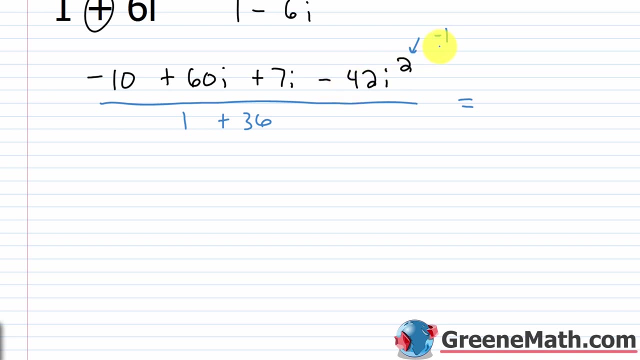 So 6, and then I would square it, that's 36.. All right, And again, if you don't believe me on that, FOIL that out and you'll see that you get the same thing. All right, so we have negative 42 times negative: 1,, which is 42,, 42 minus 10,, which is 32.. 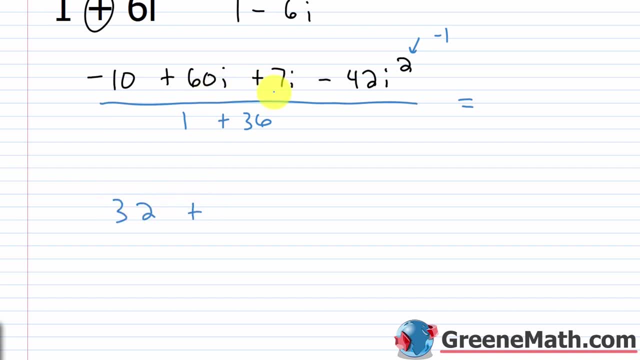 So you'll have 32, then plus 60I, plus 7I is 67I, then over 1, plus 36 is 37. So you'll end up with 32 plus 67I over 37.. 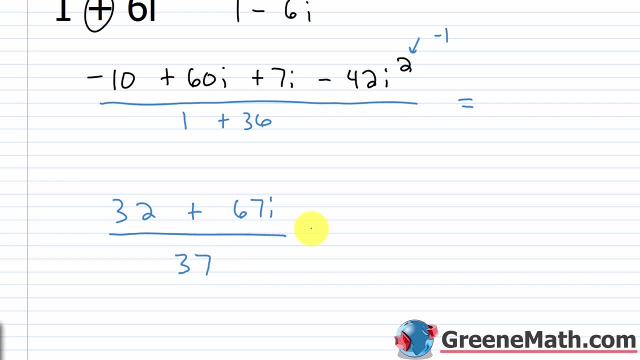 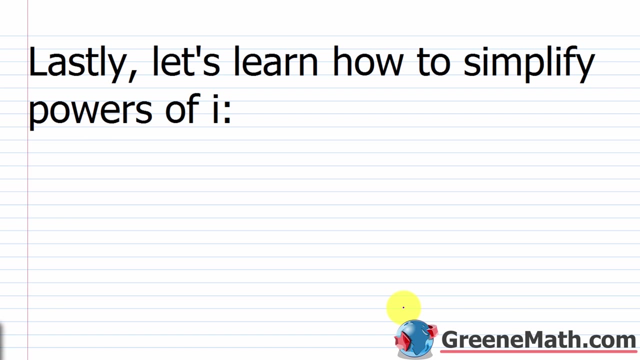 Now another thing we can do to simplify that further. another thing again: if you wanted to, you could say: this is 32 over 37 plus 67 over 37, and then times I: All right. so the last thing we want to talk about- and I know this lesson's kind of dragged on a little bit- we want to learn how to simplify powers of I. 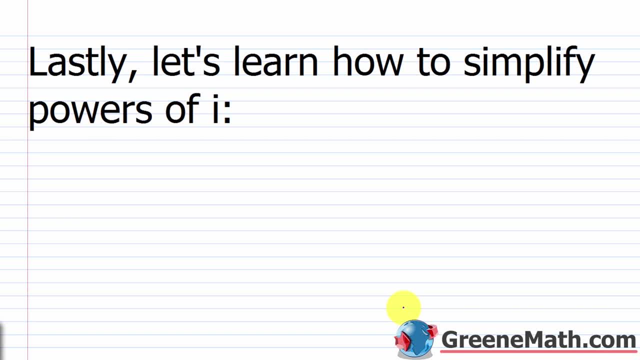 So this is something for sure you're going to see in this section, And basically it just cycles through These four values. So we start off with I to the first power, or just I. We know this is nothing more than the square root of negative 1, but we just write it as I for now. 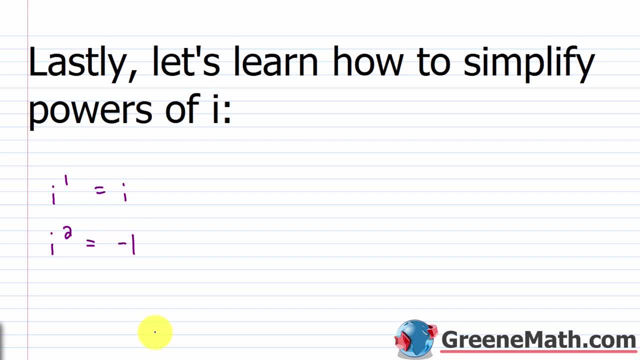 Then we see I squared. We know, by definition, this is negative 1.. Then we have I cubed. Now what is I cubed? Using the rules for exponents, it's I squared times I to the first power. I squared is negative 1.. 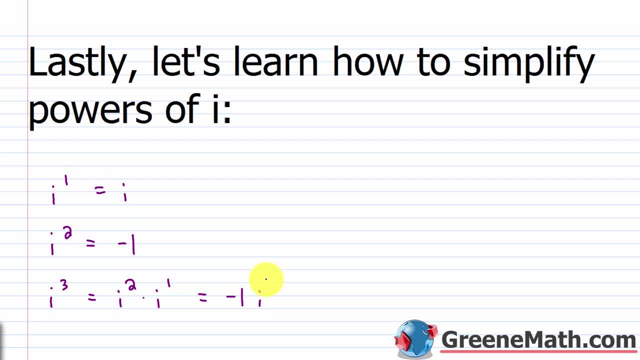 And I to. the first power I squared is just I. I mean, you could rewrite it as a square root of negative 1, but for the purposes of what we're doing here, this is just going to be equal to negative, or the negative 1, times I. 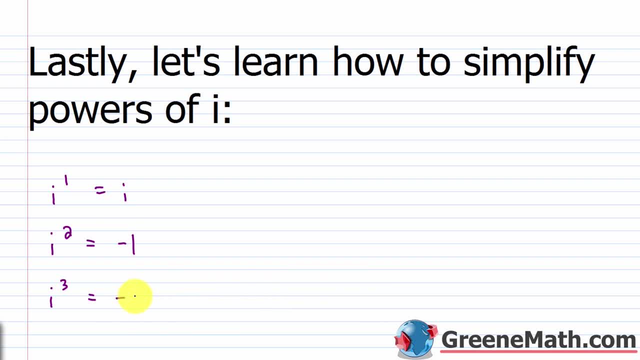 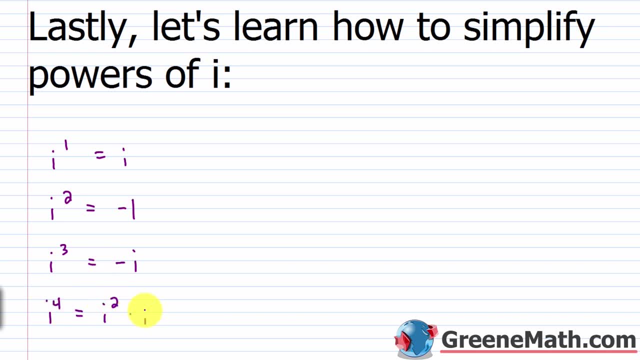 Let me erase all this and we'll make it more compact. This is just negative I. And then, lastly, we have I to the fourth power. So I to the fourth power is going to be: I squared times I squared, which is negative, 1 times negative 1, which is 1.. 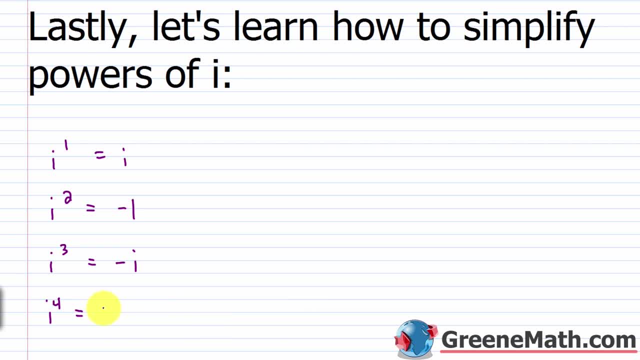 Now, when you work with something that has an exponent okay, that's larger than 4, let's say, I saw something like I to the 18th power And you get this on a test and you're like freaking out. 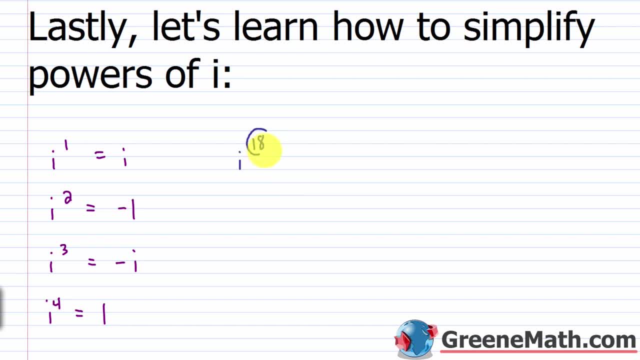 What do I do? How do I simplify that? Well, think about 18.. 18 is what. It's not divisible by 4.. I mean it's divisible by 3.. It's divisible by 2.. It's a lot of different things you can do here. 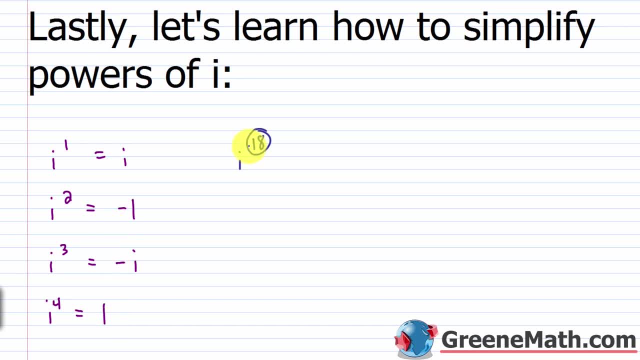 But the quickest thing to do is think about. well, 18 is 2 away from a number that is divisible by 4.. 16 is divisible by 4.. So using my rules for exponents, I could say: this is I. to the 16th power times I squared. 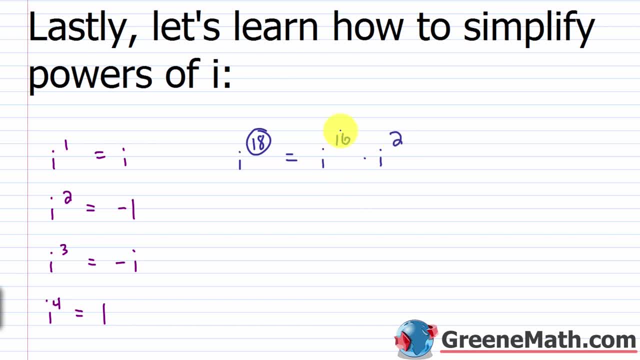 If you have I raised to a power that is divisible by 4, you can just say that hey, this is equal to 1.. It's just that quick, And the reason you can do that is to kind of go through this. 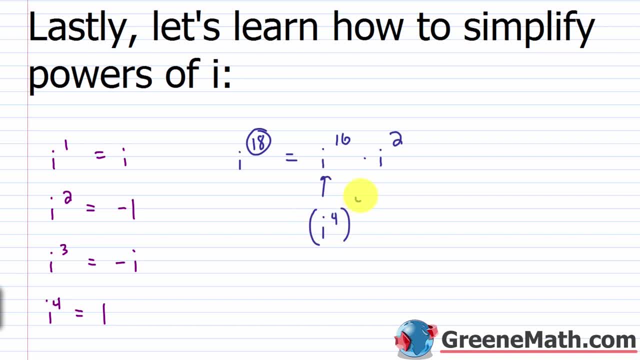 I could write this as I to the fourth power raised to the fourth power right: 4 times 4 is 16.. I've done nothing illegal. I to the fourth power, by definition, is 1.. So this is nothing more than 1 to the fourth power, which is 1.. 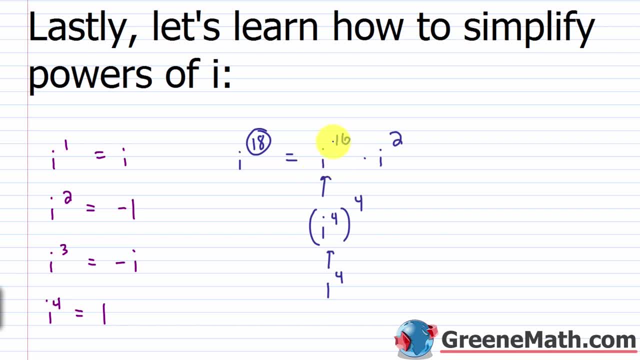 So if you have I raised to a power that's divisible by 4, you can just replace it with 1.. So this is basically 1 times I squared. Now I've simplified this to the point where I can just look at my little chart here. 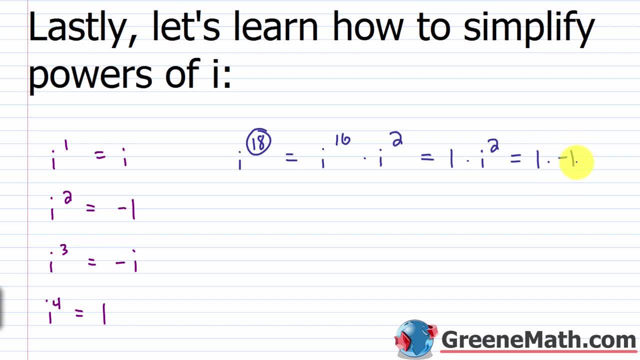 I know I squared is negative 1.. So this is 1 times negative 1, which is just negative 1.. It's really that simple. If I looked at something really, really big, let's say I saw something like I to the. 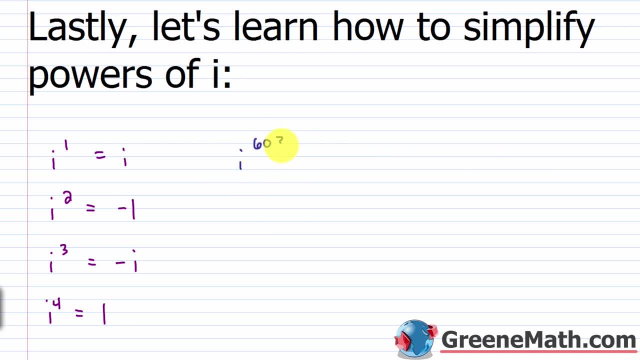 power of, I don't know. let's say 600, 3.. Well, I would know that if I came across 600, that's divisible by 4.. So I could write this as I to the power of 600 times I to the power of 3.. 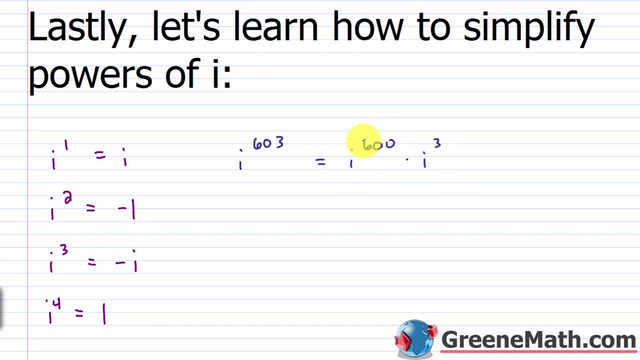 So again, if you see, I to a power that's divisible by 4, okay, 600 being divisible by 4, we can just mark it out and say this is 1.. So this is 1 times I cubed. 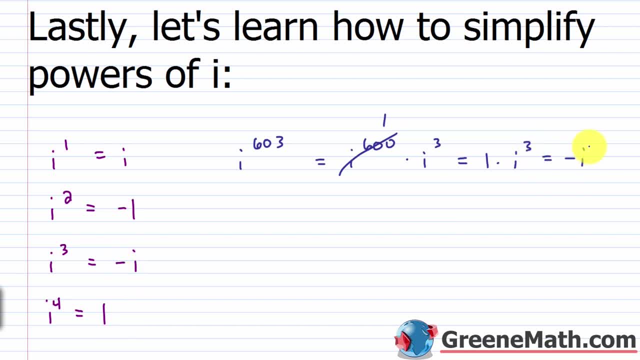 And I cubed. if I look at my little chart is negative. I Okay, very, very simple. As another example, let's say that we looked at something like a negative exponent. Let's say negative, I don't know. let's say 9.. 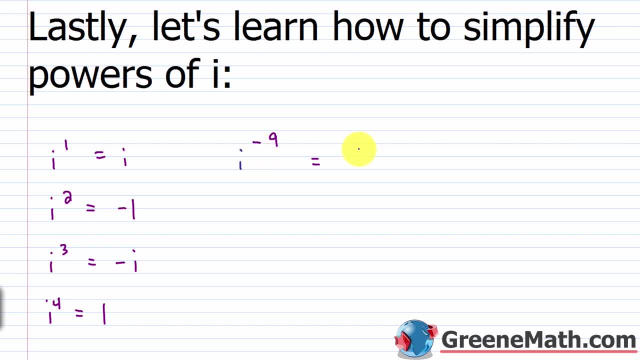 So what do we do? We know, with negative exponents we write 1 over I to the 9th power. So same rules apply here. We think about simplifying this. So 9 is what? If you think about 9, 1 less would be 8.. 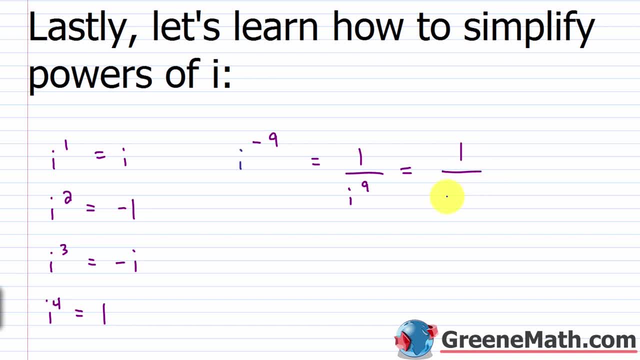 8 is divisible by 4.. So let's go ahead and do that. We have: I to the 8th power times. I. I to the 8th power. again, if 8 is divisible by 4, you can mark this out and just put 1.. 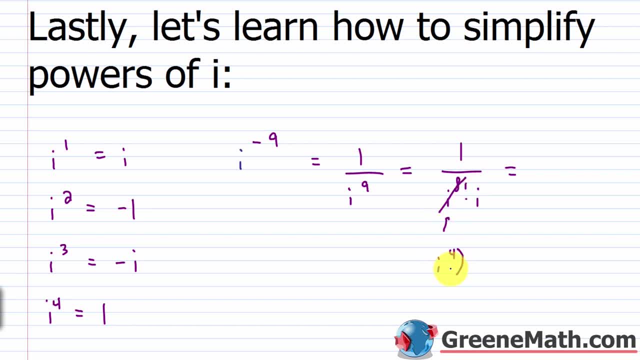 Because I can always just say: this is I to the 4th power, squared I to the 4th, power is 1.. 1, squared is just 1.. So any time you get I raised to a power and that power is divisible by 4,. 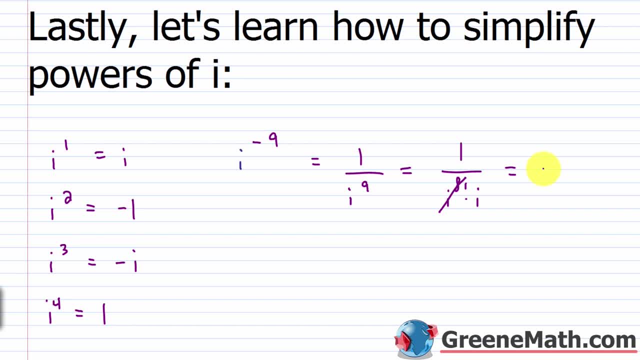 cross it out and just put 1.. Okay, that's all you got to do. So what I'm left with is a 1 over I. Again, this represents the square root of negative 1.. So we rationalize something like this: 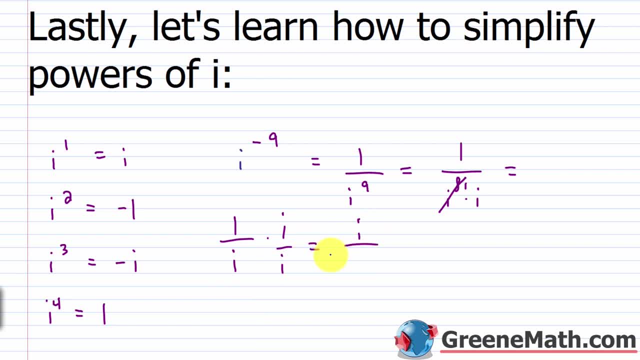 So times I over I, You would get I over I. times I is I squared, which is negative 1, which equals negative I. And again, this is a more complex problem that you might see. A lot of students will get this far. 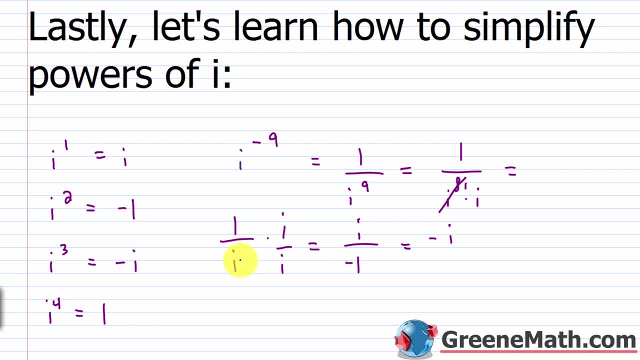 Okay, they'll get 1 over I, but they won't take the extra step of rationalizing the denominator to get this negative I as a result. So this right here, although it's not technically wrong, it's not how we report our answer. 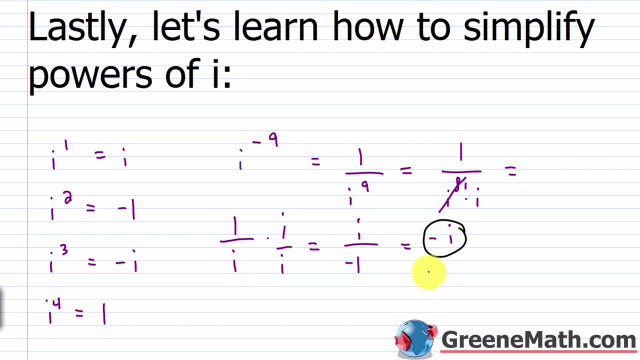 And so you will get marked off on the test for that. Okay, so you've got to make sure you report this and not just that. All right, let's take a look at another one. Let's say we had I don't know. let's say I to the power of 57.. 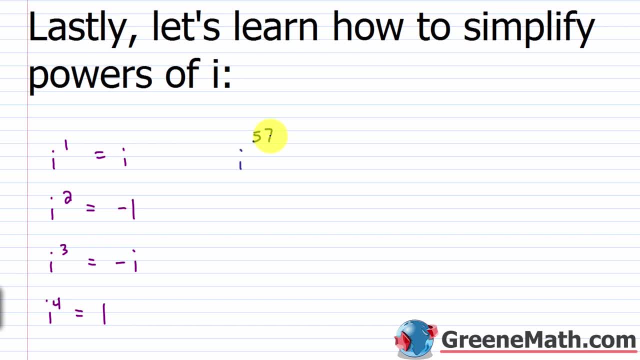 Well, we know that 57 is divisible by 3.. So would we want to do that or would we want to do this? Let me ask you what's better. Should I go? I to the 56th power. 56 is divisible by 4,. 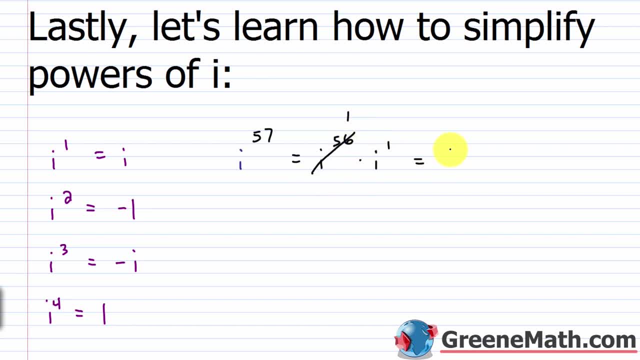 times I to the first power. We know this would be 1, so this is 1 times I, or just I. That was very quick, Let's say I said: okay, well, I know I cubed is negative. I Let's try it this way. 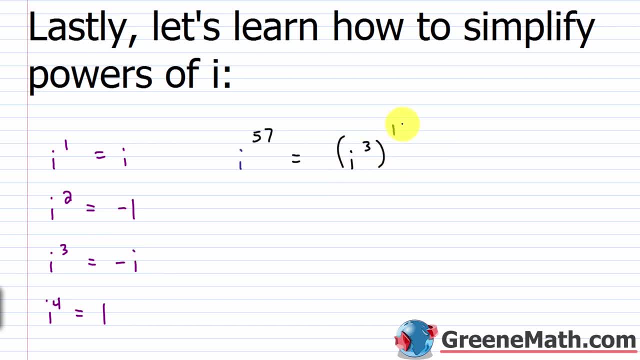 Let's say this: is I cubed, raised to the power of 19.. Is that going to get me anywhere? Really, all this is telling me is I have negative I raised to the 19th power. Does that get me where I want to go? 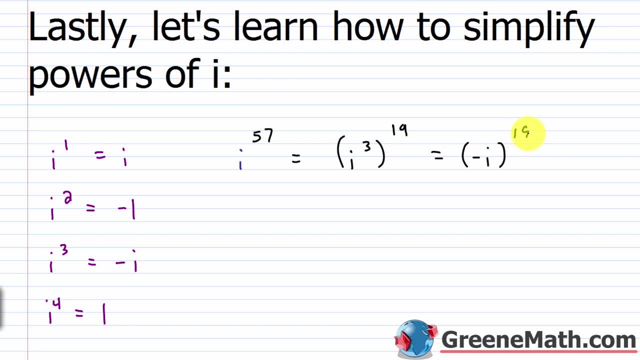 No, it really doesn't Okay. If I want to do that, I want to stick to things that are going to be very, very easy, because, although I can figure this out, I can say this is negative: 1 to the 19th power times, I to the 19th power. 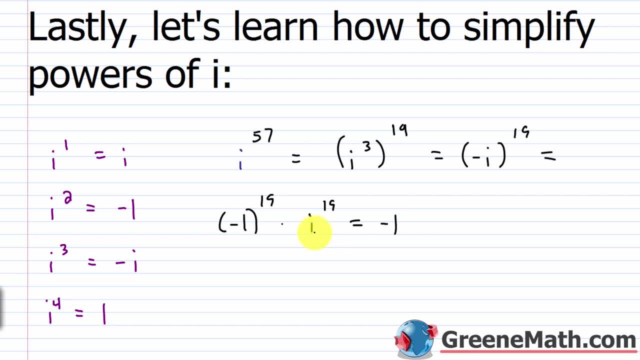 Where does that really get me? Negative? 1 to the 19th power is still negative. 1.. I to the 19th power is 1.. Well, I'm going to have to split this up. I could say it's I to the 16th power. 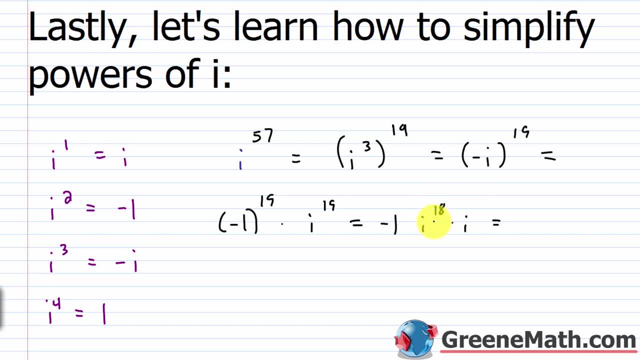 We can even do 18th power times. I Now what I'm doing here. I to the 18th power. I could say this is negative 1 times I squared to the 19th power times we'll have I. So what do we end up with? 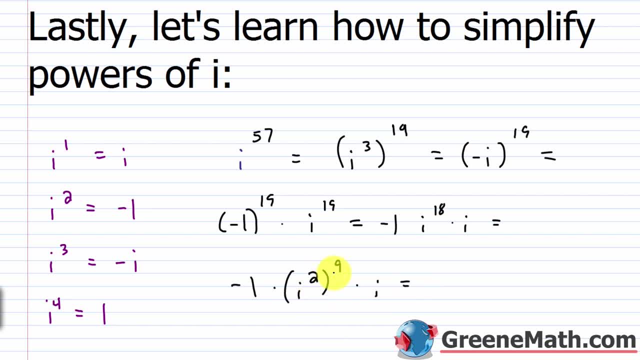 I squared is negative 1.. Negative 1 to the 19th power is still negative 1.. So you'd have negative 1 times negative 1 times I. Negative 1 times negative 1 is 1.. 1 times I is I. 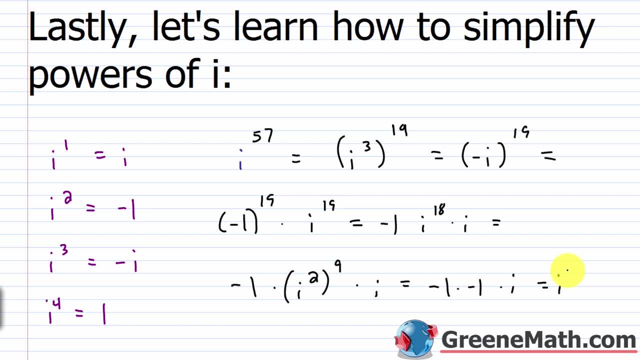 Look at all that work I had to do to figure out what I figured out very quickly by. just let me erase this real quick and I'll go back to what I just did, in case you forgot, By using the divisibility rules for 4,. 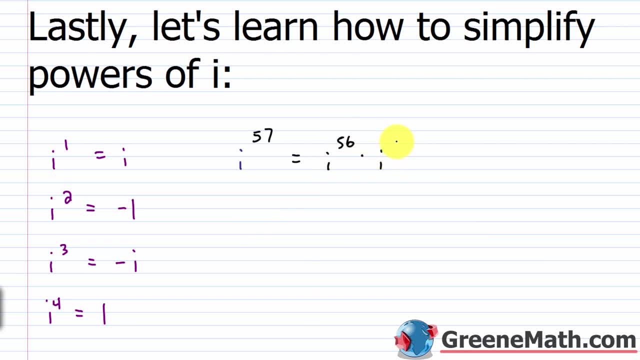 if I just said, okay, I to the 56 times, I to the first, this is 1 times, just I, So 1 times I gives me. I Look how quick that was versus what we just did. Okay, so don't make that mistake that a lot of students make. 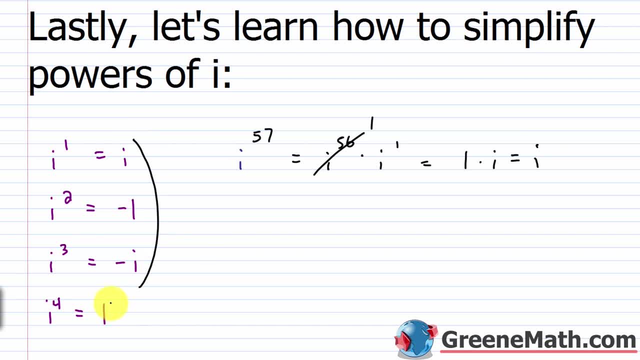 Try not to use these unless you need to. If it's a number for your exponent that's larger than 4, look for the next number down that's divisible by 4.. So if it's 13.. I'm looking to write this as I to the 12th power times. I to the first power. 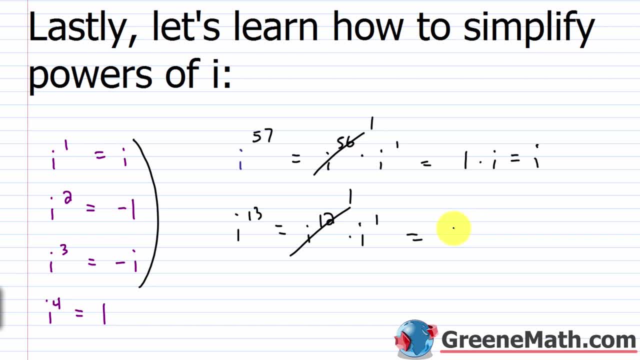 This is 1 and you get 1 times I. If it's I to the 49th power, we know 48 is divisible by 4.. So I to the 48th power times. I to the first power. This is 1.. 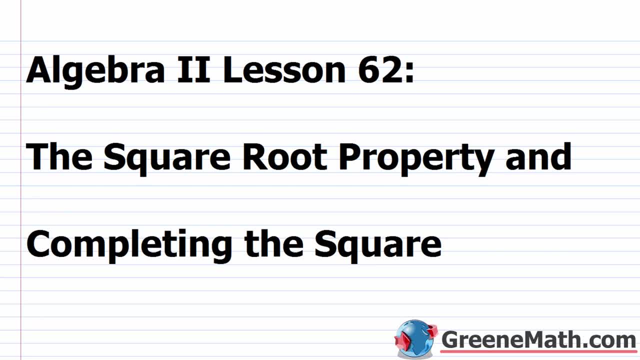 1 times. I is just I. Hello and welcome to Algebra 2, Lesson 62.. In this video, we're going to learn about the square root property and completing the square, So I want you to recall that a quadratic equation has a squared term. 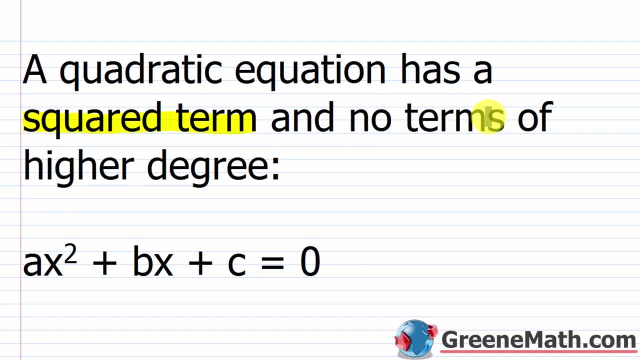 Okay, a squared term and then no terms of higher degree. So, as a generic example, one that you'll probably see in your textbook, we have ax squared. Let me highlight that exponent of 2 plus bx plus c equals 0. So this is a quadratic equation. 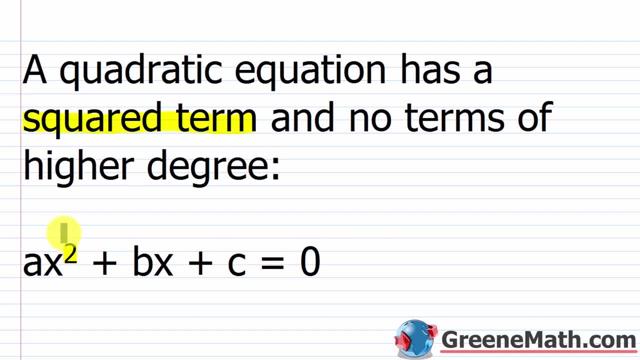 in standard form. So you'll see that the exponents go in descending order. You have the exponent that's 2 and you have the exponent that's 1.. And one thing you need to understand here is that for a, b and c, 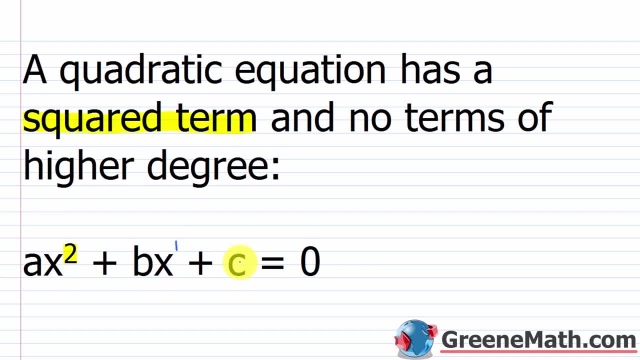 a is the coefficient of x squared, b is the coefficient of x and c is the constant. They're allowed to be any real number that you want, with one exception: A- the coefficient of x squared is not allowed to be equal to 0.. 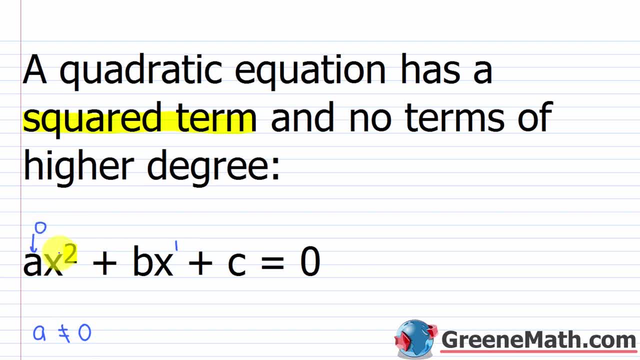 Because if we plugged in a 0 there you'd have 0 times x squared, So that term would basically go away. You'd be left with bx plus c equals 0. So without a squared term there it would no longer be a quadratic equation. 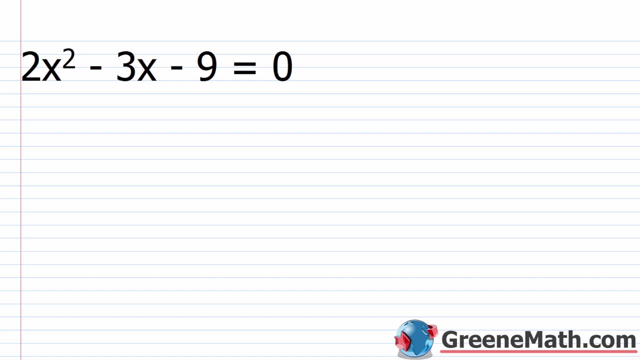 And so that's why that's not allowed. We previously learned how to solve a quadratic equation by factoring, And, for those of you that took an Algebra 1 course, you've already learned how to solve a quadratic equation by using this process, known as completing the square. 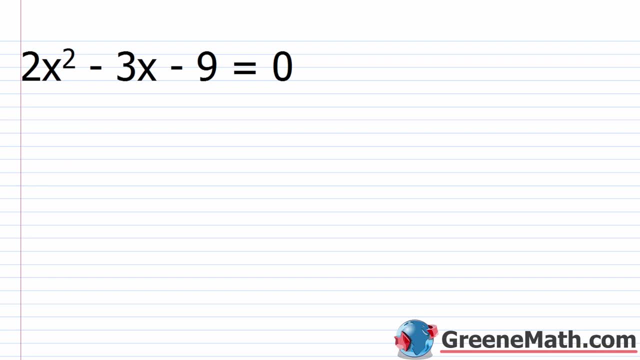 And then more easily using a process known as the quadratic formula. So basically we're going to go through that again. Hopefully you did see it in Algebra 1 and this is just a refresher. If you didn't, it's not too hard to pick this up here. 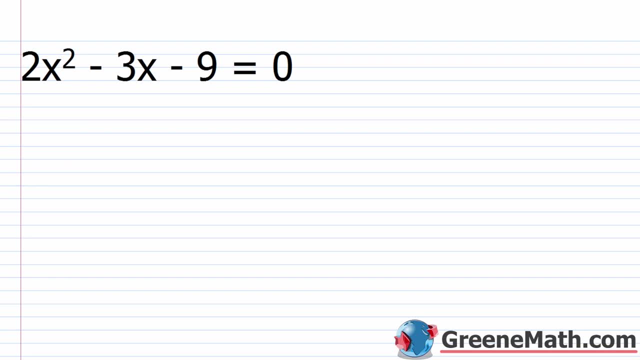 So we're going to start out by just going through what to do when it is factorable. So we have 2x squared minus 3x minus 9 equals 0. So what we want to do is we want to factor the left side. 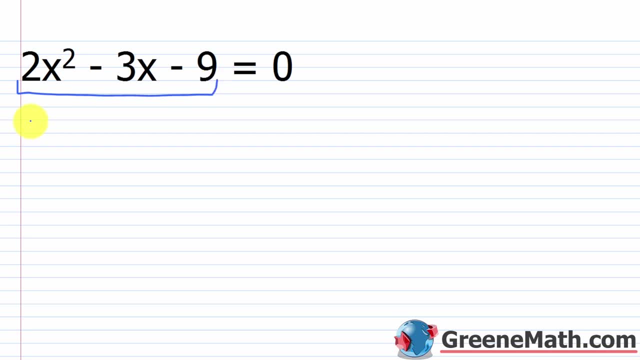 So we know how to factor a trinomial into the product of two binomials. Now, at this point in Algebra 2, you should have a preferred method for doing this. Either it's reverse FOIL or it's factoring by grouping. whatever you want to do. 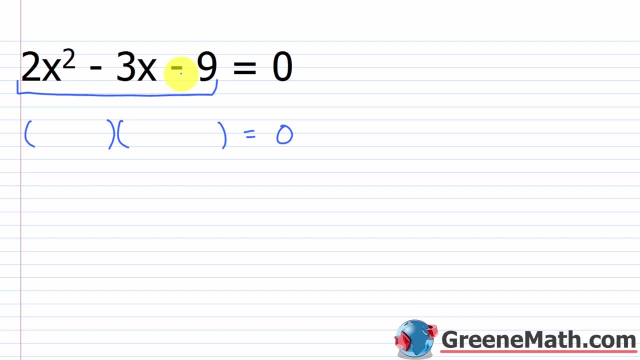 For myself. I see that this is pretty easy to do with reverse FOIL. You have 2,, which is a prime number, times x squared, So I know that's going to factor into 2x and then x. So I know those first two positions. 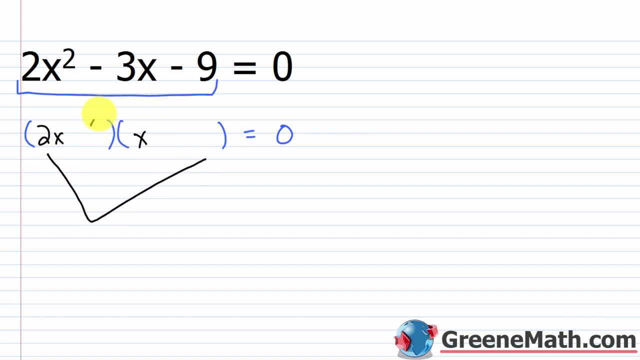 I just need to work out the outer and the inner. to sum to this term: negative 3x. So the way you do that is: you look at negative 9 and you say: well, what are the possible factors of negative 9?? Well, it's negative 1 and positive 9, or it's positive 1 and negative 9.. 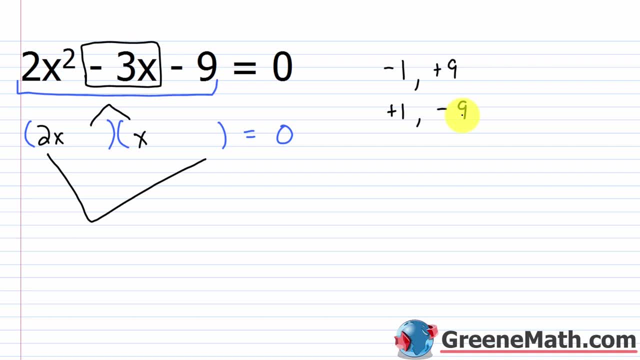 The only thing is, those would never work out for you, And the reason for that is they're too far apart. If I put a positive 9 here and a negative 1, you'd end up with an outer of 18x and an inner of negative x. 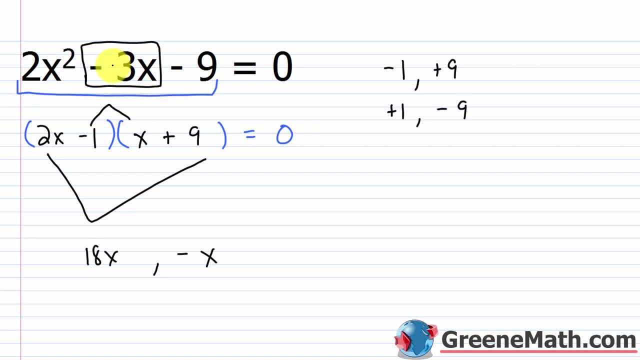 Those are too far apart to ever give you a negative 3x in terms of a sum. If I flip the signs around and I did positive 1 and I did negative 9, it's going to be the same thing. It's just too far away. 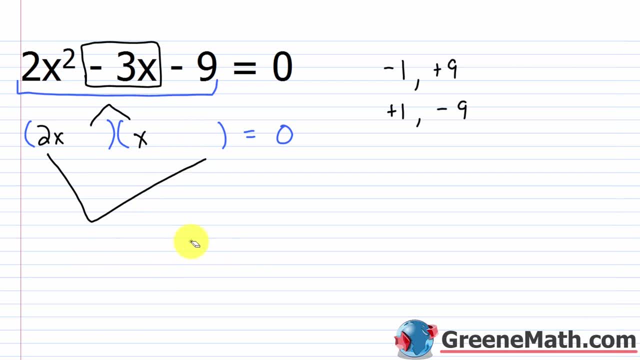 So we can go ahead and eliminate those and say that those are not going to work. Okay, so what would work? Well, in terms of negative 9, you have another possibility. You have positive 3.. You have positive 3 and you have negative 3.. 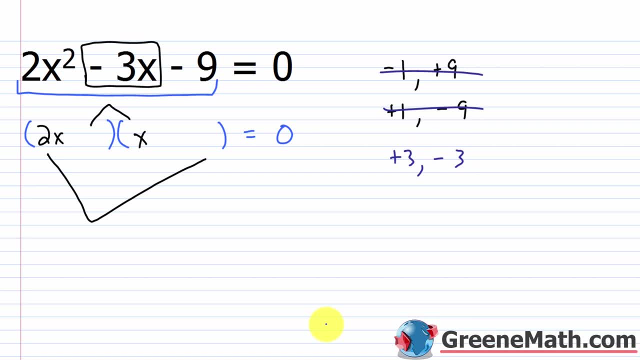 Now, where would I want to put negative 3?? Where would I want to put positive 3?? If the result here is a negative 3x, I want the term that's going to be larger in terms of absolute value to be negative. 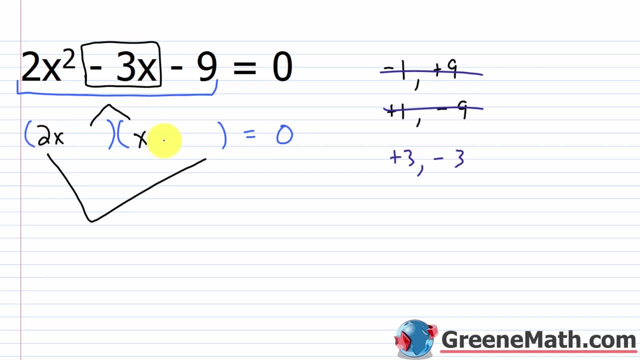 So I would think about the 2x multiplying by the negative 3.. And I would think about the 1x multiplying by the positive 3, so that my result again, when I do the sum, is going to be negative. And we can check this, We do our FOIL. 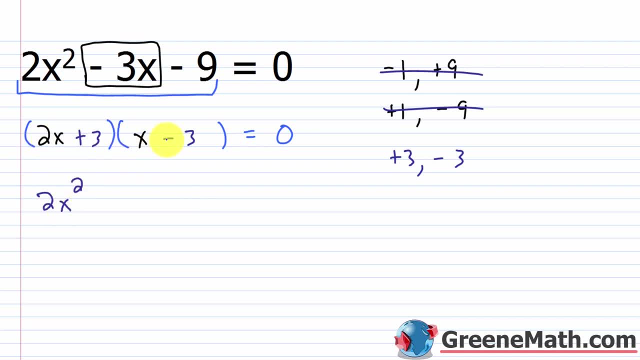 2x times x is 2x squared. My outer 2x times negative 3 would be minus 6x. My inner 3 times x would be plus 3x. And then my last 3 times negative, 3 is negative 9.. 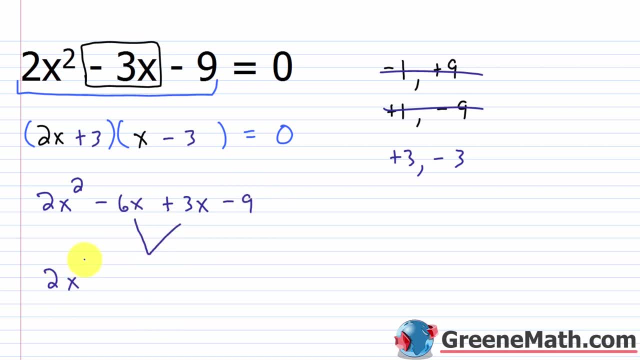 So if you sum these two now, you would have 2x squared minus 3x minus 9, which is exactly what we started with right here. The main thing here- let me just erase this- is just to understand how we go about solving this by factor. 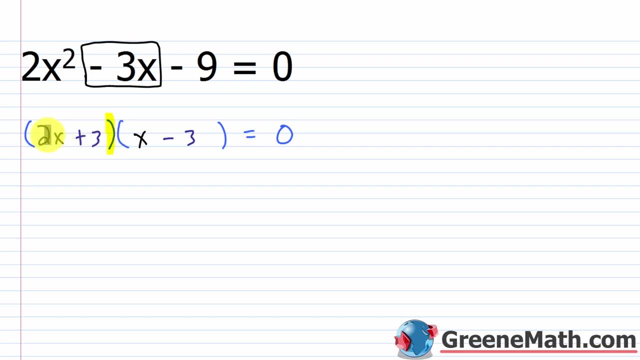 I want you to realize that this right here inside of parentheses, is a factor, and so is this. It's one of the hardest things for students to wrap their head around. This is multiplication. here, The quantity 2x plus 3 is multiplied by the quantity x minus 3, and this equals 0.. 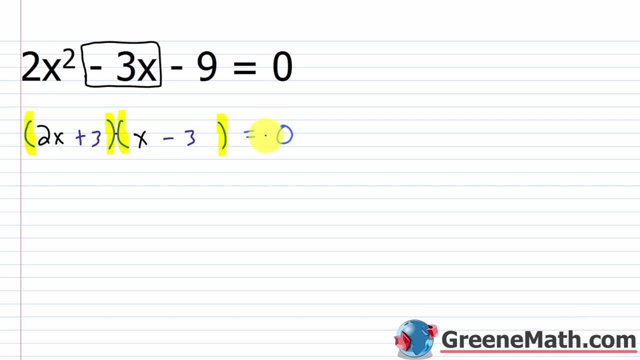 So we use something known as the zero product property. What does that tell us? Well, if you have something like a times b and this equals 0, well, what are the possibilities? We know, when we multiply by 0, we get 0 as a result. 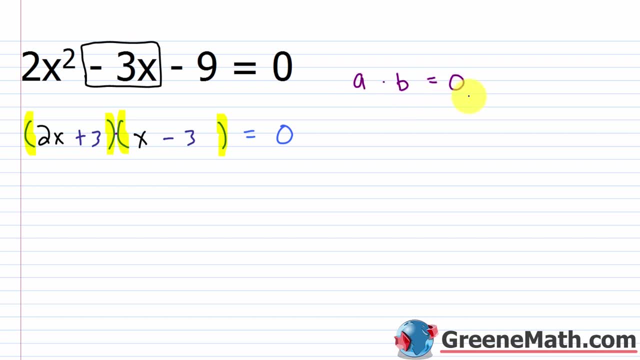 So either a is 0, b is 0, or they're both 0. It's got to be one of those things. So what I can do is I can extend that here and say: well, either 2x plus 3 is equal to 0, or this other factor here, x minus 3 is equal to 0. 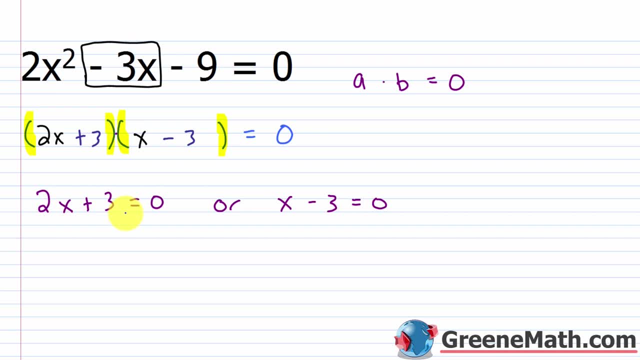 So when we solve each equation here separately- so I would subtract 3 away from each side of this equation- we would get 2x is equal to negative 3. Then when we divide both sides by 2, then we would get x is equal to negative 3 halves. 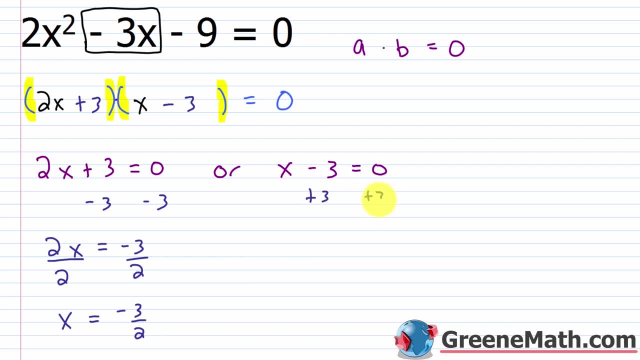 Then over here we add 3 to each side of the equation and we would have: x is equal to 3.. So you have two solutions here: x equals negative 3 halves, or x equals 3.. Let me just kind of notate that up here. 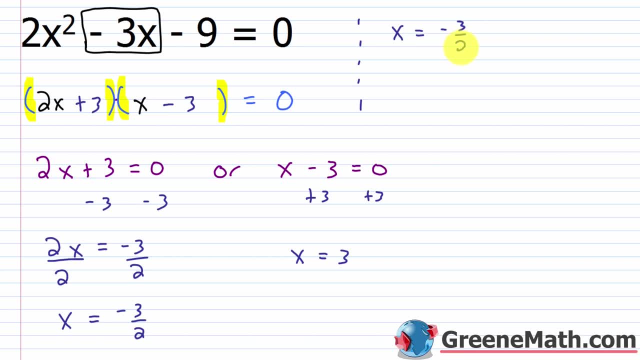 We'll say x is equal to negative 3 halves, Or x is equal to 3.. Using solution set notation, we could put negative 3 halves, comma 3.. Now, if you wanted to, you could pause the video at this point. 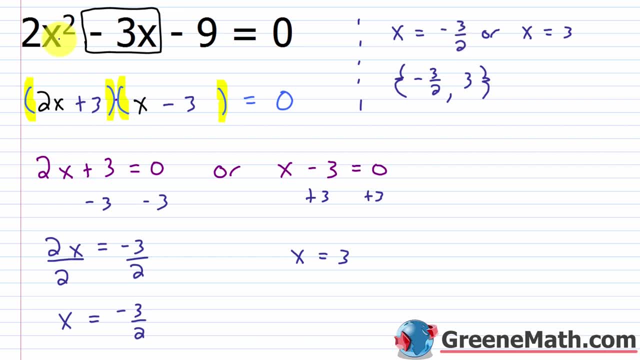 and you could stop and you could check these. You could plug a negative 3 halves in for each x and verify that you get the same value on both sides of the equation. In this case it would be 0 equals 0.. You could also plug in a 3 and verify that you get 0 equals 0. 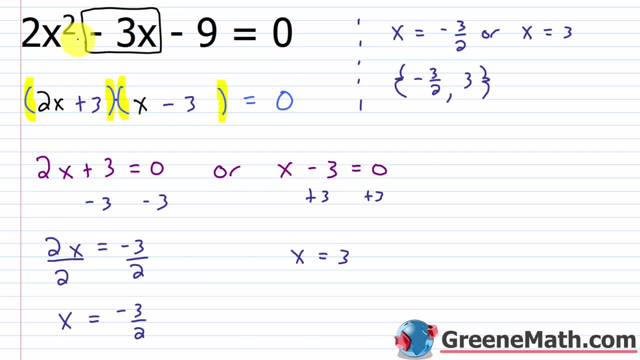 I'll leave that up to you to do on your own. What I want to do now is talk about what can we do when we can't solve a quadratic equation by factoring. Well, again, we have a few different methods available, And we're going to start out by just talking about something known as the square root property. 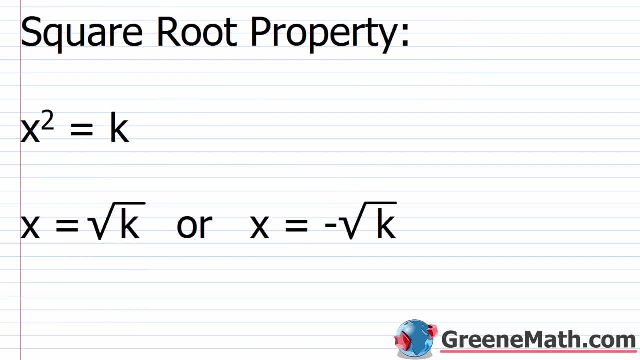 So here's the square root property And again, if you took Algebra 1, you'll remember this- It tells us that if x squared is equal to k, then x is equal to the square root of k or x is equal to the negative square root of k. 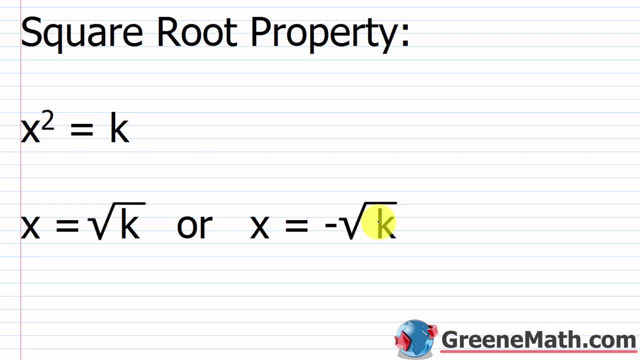 Remember, we have those two different notations. This is the principal square root and this is the negative square root. You might say: well, why do you need that? Well, just think about if you had something like x squared is equal to 4.. 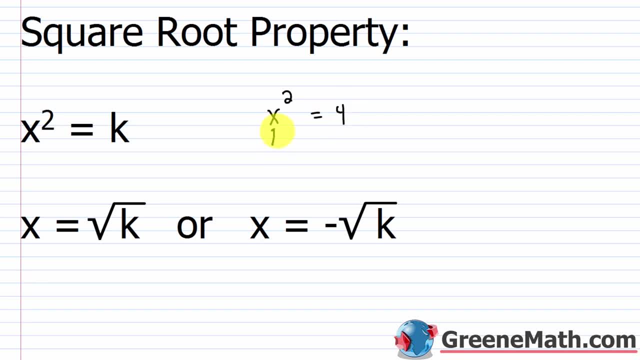 We all know at this point that I could plug in a 2 there and say 2 squared is equal to 4, so that would be a solution. Or I could also plug in a negative 2 there and say negative 2 squared is equal to 4.. 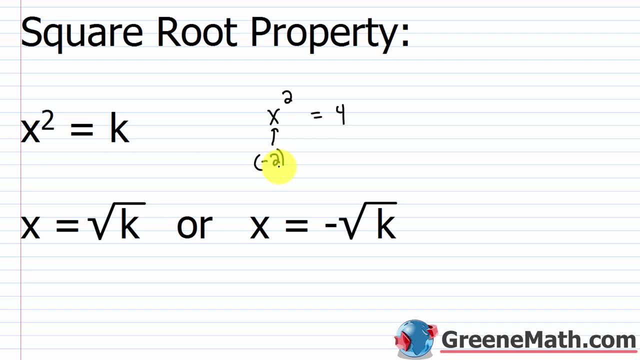 The real thing is here: when you square something, you lose that information about the sign. Was it positive? Was it negative? Because both of them would work and you really don't know. So you have to account for both possibilities And you say x is equal to the principal square root of k. 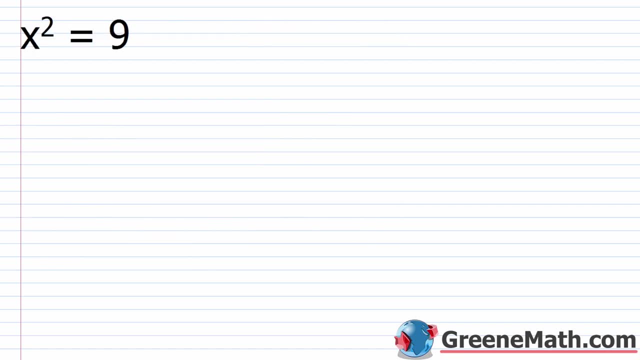 or x is equal to the negative square root of k. So here's another good example. Let's say we saw something like x squared is equal to 9.. So x squared is equal to 9.. So what we would do is we would take the square root of this side. 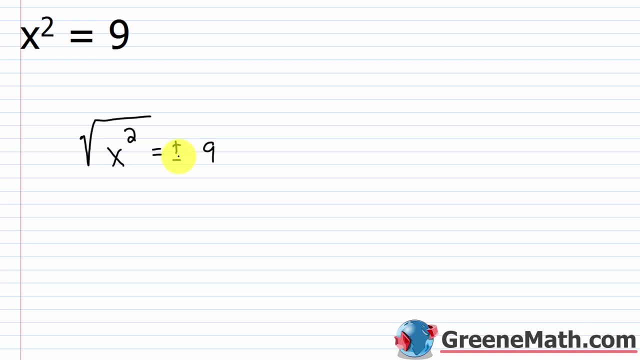 and then we would say plus or minus. This is shorthand for saying positive square root or principal square root or negative square root. You put plus and then you put a minus sign underneath And then we'll say the square root of 9.. 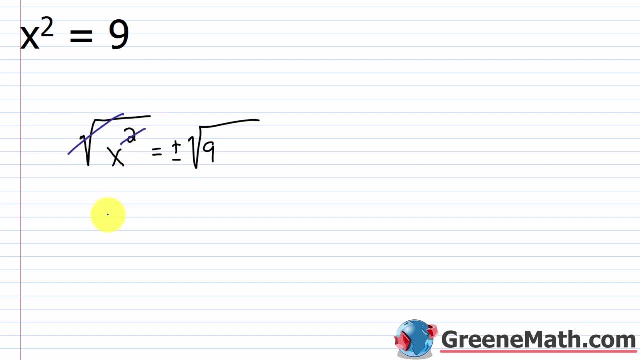 So we all know at this point that this would cancel with this and we would just have x by itself. And this equals plus or minus the square root of 9,, which is 3.. Now, don't get fooled here. This is two different solutions. 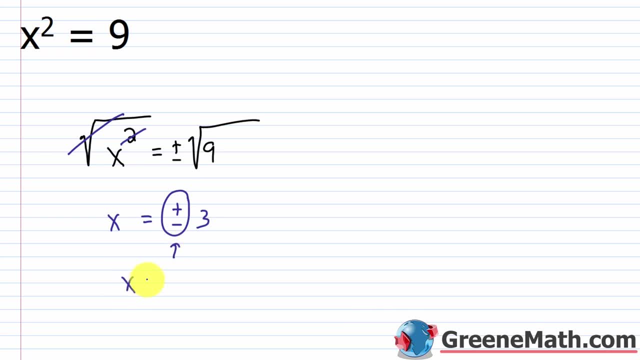 This tells me right here that I have: x is equal to positive 3, or x is equal to negative 3.. Again, if I plugged in a 3 here and I squared it, I'd get 9.. If I plugged in a negative 3 and squared it, I'd also get 9.. 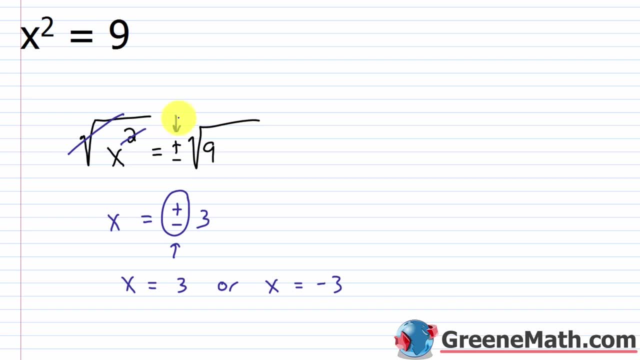 So we're counting for both of those possibilities with this plus or minus here. All right, so let's take a look at an example that we can use this on. So we have 4x squared plus 2 equals 102.. So you might say, whoa, that doesn't look like something I'd use the square root property on. 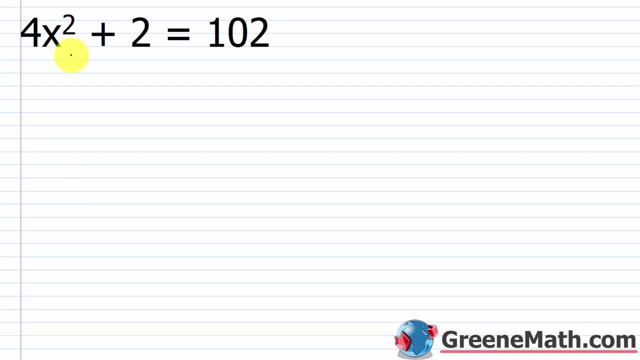 If you have a perfect square equal to some number, you can use the square root property immediately. Now we don't have that here, but we could easily do that if we just subtract 2 away from each side, And then we would have what We would have. 4x squared is equal to 100.. 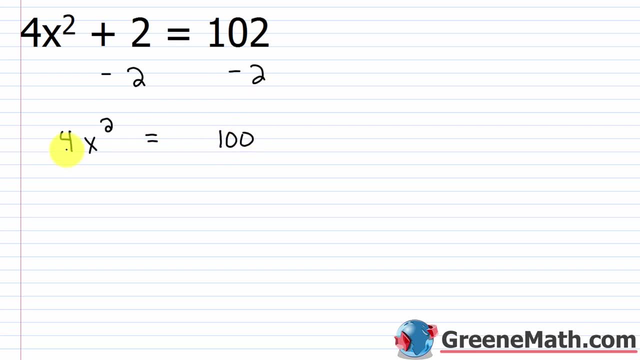 Now you have the option. 4 is a perfect square, But typically it's a little bit easier if you just have a coefficient of 1 here. So let's go ahead and just divide both sides of the equation by 4. And we'll find that x squared is equal to 25.. 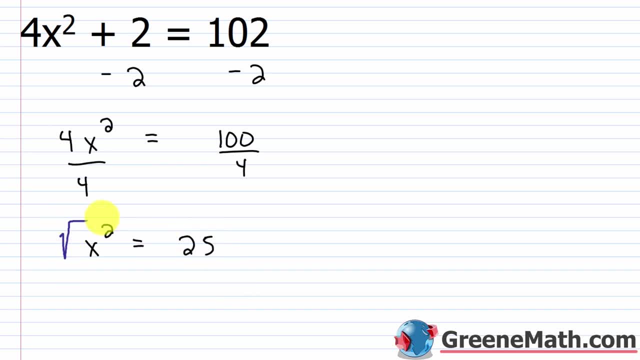 And then if we use our square root property, we could say: take the square root of this side and then plus or minus the square root of this side. So this would be: x is equal to plus or minus 5, right Square root of 25 is 5.. 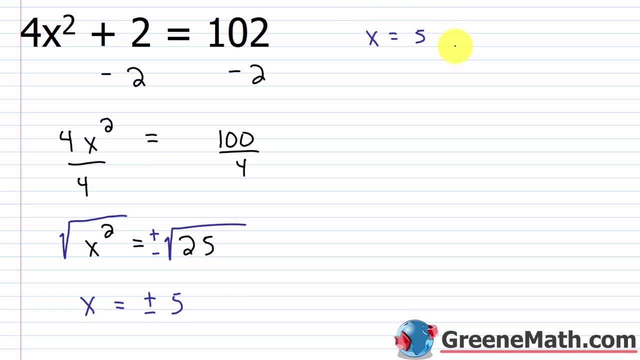 So again, this is two solutions. This is x is equal to 5 or x is equal to negative 5.. So we can write negative 5, comma 5, like that. And for this one let's just stop and check for a second. 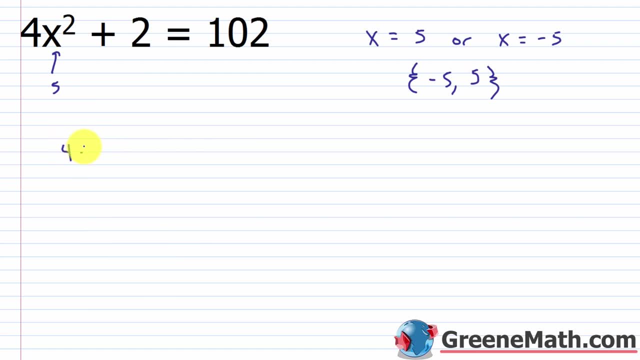 So if I plugged in a 5 there, what would we get? You'd have: 4 times 5, squared is 25, then plus 2 equals 102.. Yeah, 4 times 25 is 100.. 100 plus 2 is 102.. 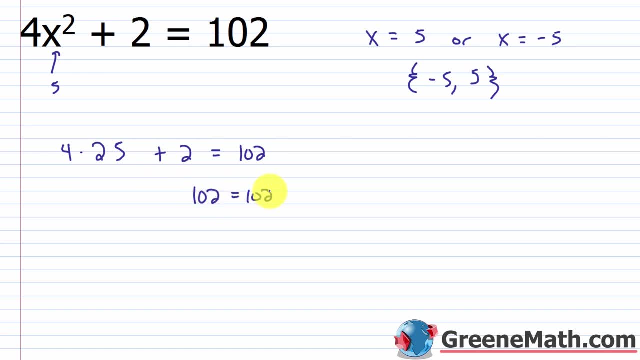 You'd end up with 102 equals 102.. And again, if I plugged in a negative 5, it would be no different. Negative 5 squared is also 25, so it leads to this exact same scenario. Now let's try without dividing both sides by 4.. 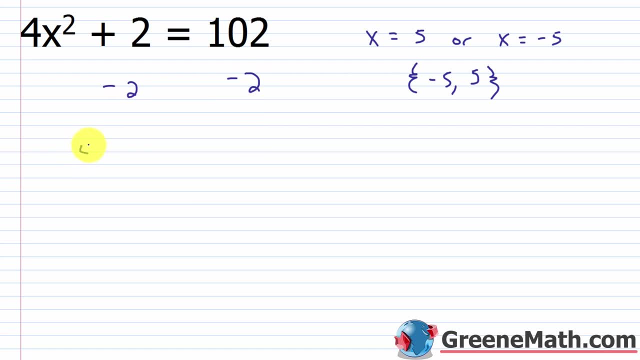 If we just subtracted 2 away from each side of the equation, we'd have 4x. squared is equal to 100.. What happens if I take the square root of this side and I go plus or minus the square root of this side? 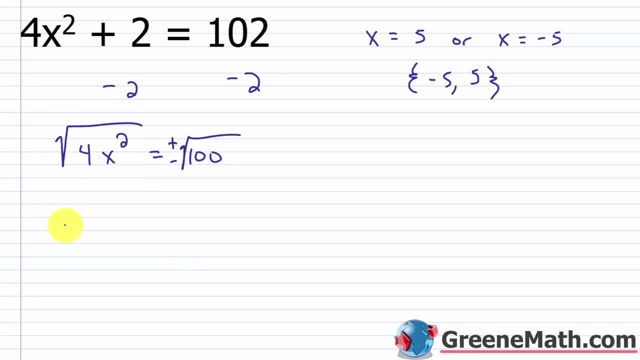 Well, the square root of 4 is 2.. The square root of x squared is x, so I'd have: 2x is equal to plus or minus the square root of 100, which we might as well just say plus or minus 10.. 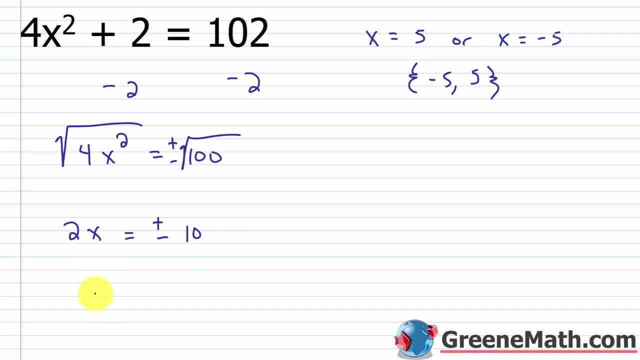 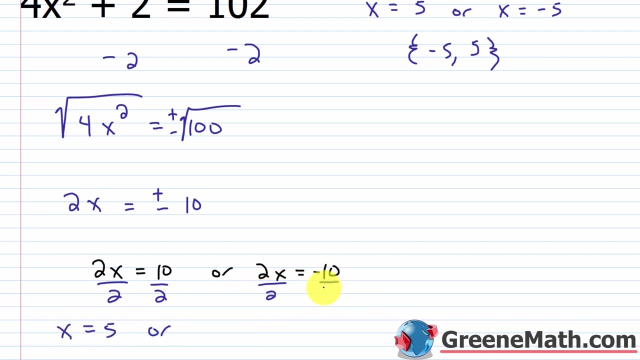 Now this leads to two different equations. It's 2x is equal to 10 or 2x is equal to negative 10.. If you solve these for x, we divide both sides by 2, you're going to get x is equal to 5, or divide both sides by 2 here. 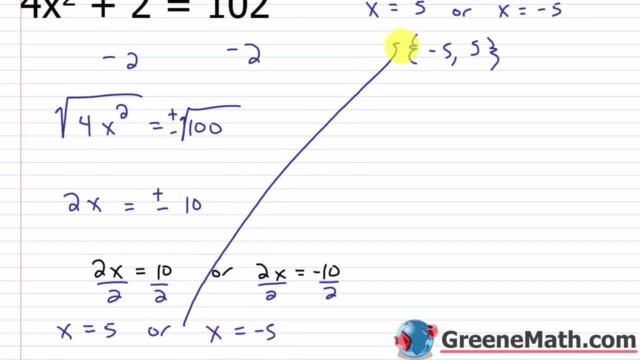 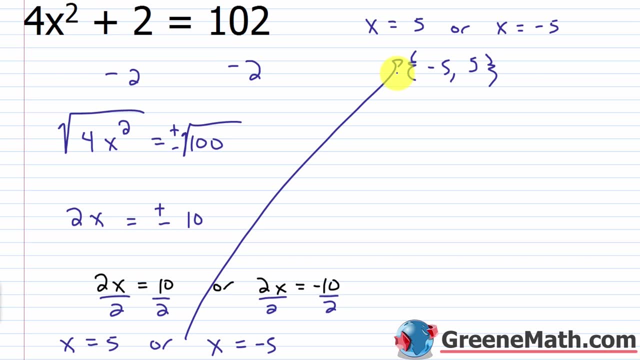 you'll get. x is equal to negative 5.. Again, exact same thing. I got there. It's just a little quicker, because we divided both sides by 4, okay, And we got x squared by itself. So you pretty much want to do that to save yourself the extra work. 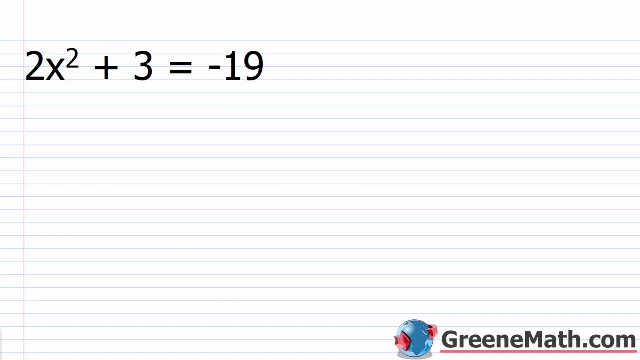 that we had to do here. All right, let's take a look at another one. So we have 2x squared plus 3 equals negative 19. So again, if I have something squared equal to a number, I can use that square root property. 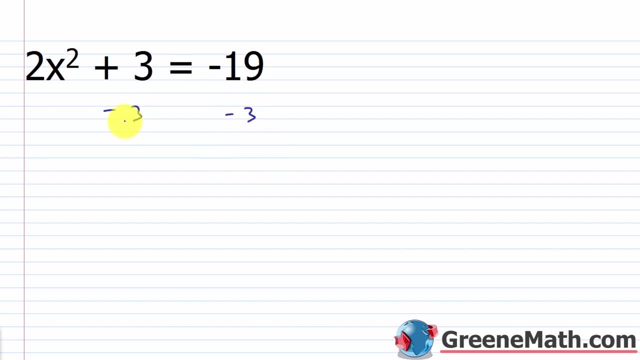 So let me subtract 3 away from each side of the equation, So that'll go away. We'll have: 2x squared is equal to negative. 19 minus 3 is negative 22.. I want x squared by itself. I want 1x squared. 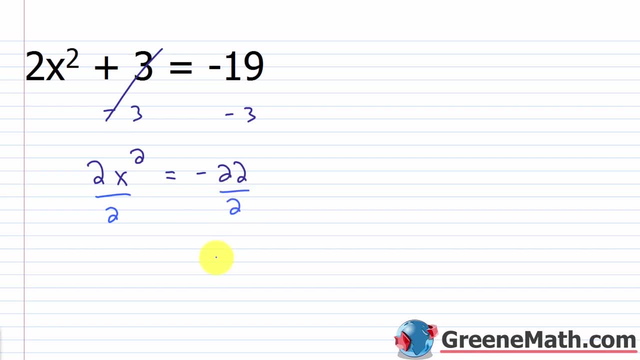 So let's divide both sides of the equation by 2. And this will cancel. with this We'll have x squared is equal to negative 11. And then now all I need to do is take the square root of each side. So I'll take the square root of this side. 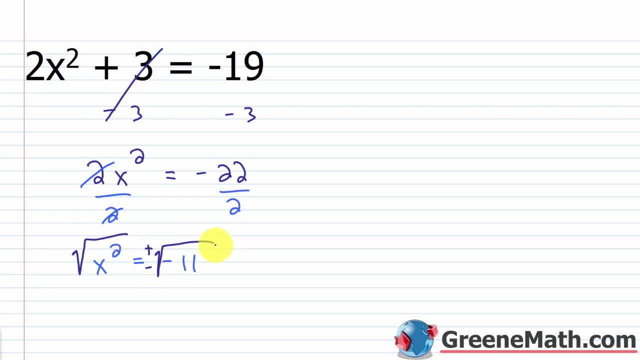 and I'll go plus or minus the square root of this side. So we know this ends up being x and this is equal to plus or minus the square root of negative 11.. Now we didn't work with negative square roots back in Algebra 1,. 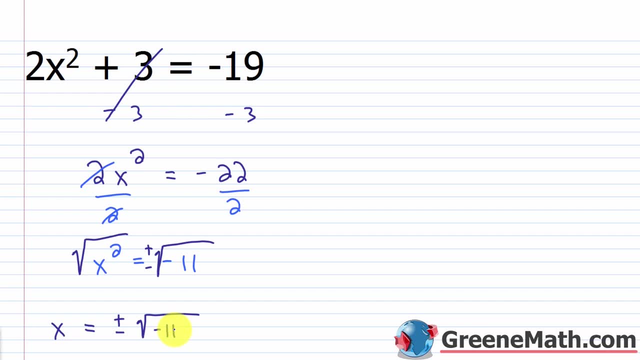 but here we've already done a lesson where we talked about this. I can say that this is: x is equal to the principal square root of negative 11, or x is equal to the negative square root of negative 11.. Now, when we think about this, 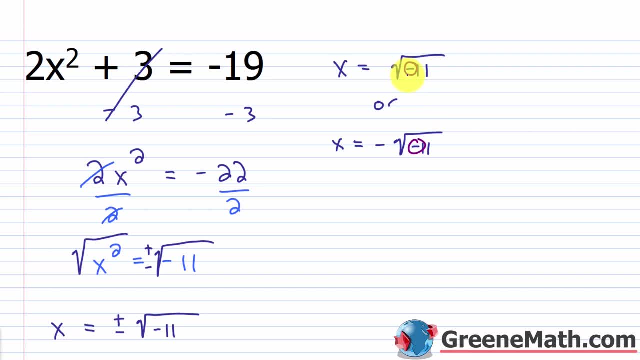 we know that if you have a negative inside, you can pull it out and just say: this is i, So I can erase that negative and I can say this is i times the square root of 11.. I can erase this negative and I can say this is negative, i times the square root of 11.. 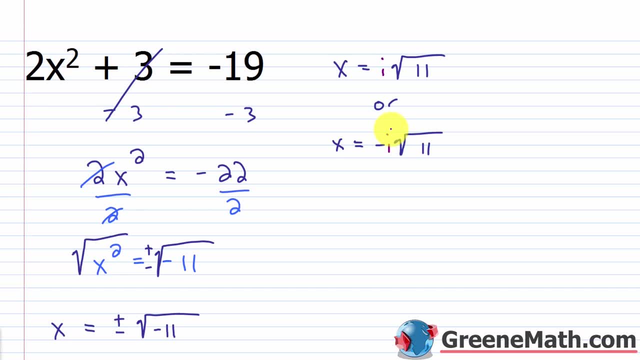 Now what if I check this to prove it to you- And I want to do that real fast, So let's just go with this first. You'd have 2 times x is squared. This whole thing is what x is equal to. 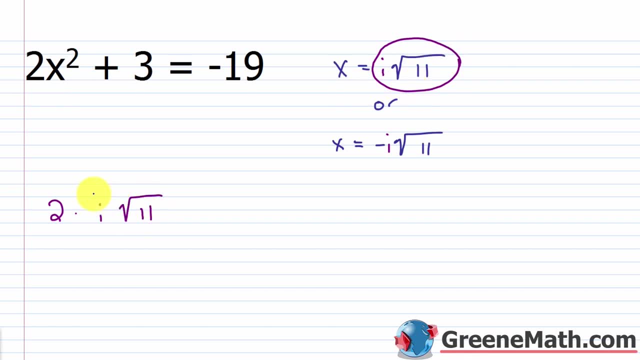 So you'd have: i times the square root of 11, and this is all squared. Then plus 3 equals negative 19.. So you'd have 2 times i squared has a definition of negative 1.. Let's just write: i squared for right now. 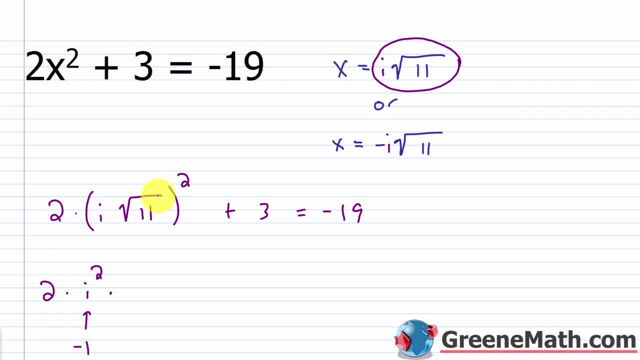 I'm just going to put an arrow and say this is negative 1.. Times the square root of 11, squared is 11.. Then plus 3 equals negative 19.. Again, I know this is negative 1.. So 2 times negative 1 is negative 2.. 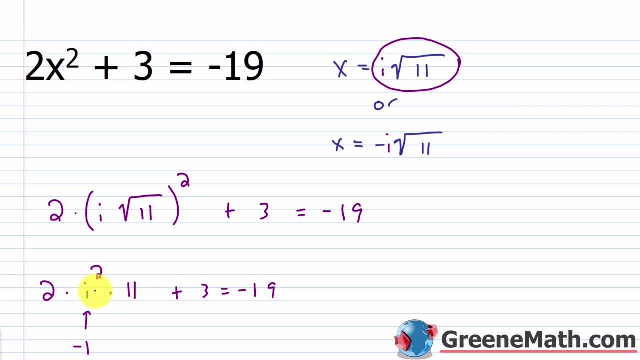 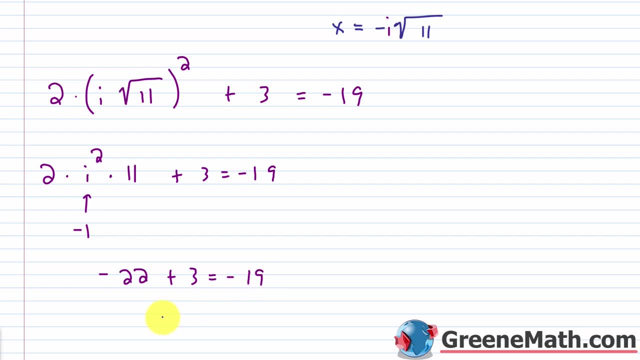 Negative 2 times 11 is negative 22.. So essentially what you have here is negative 22 plus 3 equals negative 19.. So you end up with negative 19 equals negative 19.. So yeah, that works out. Let's erase this real quick. 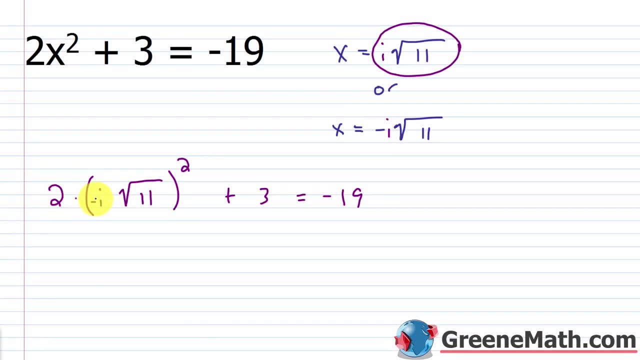 And what would happen if I had a negative? i there, if I had a negative there, Well, it wouldn't matter, because if I squared that negative I'd get a positive. It would lead to the exact same scenario where I end up with negative 19 on this side. 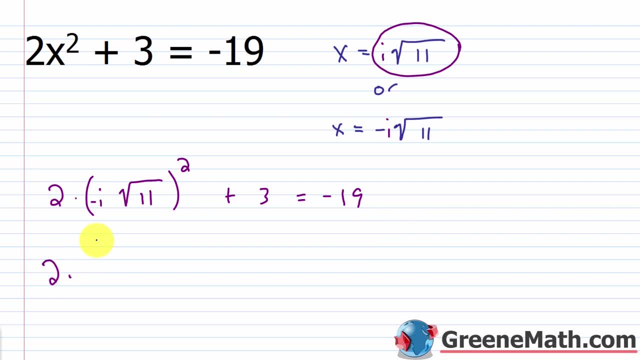 and negative 19 on this side, Again 2 times. you can think of this as negative 1 squared, which would be 1, times i squared, which is negative, 1, times the square root of 11 squared, which is 11,. 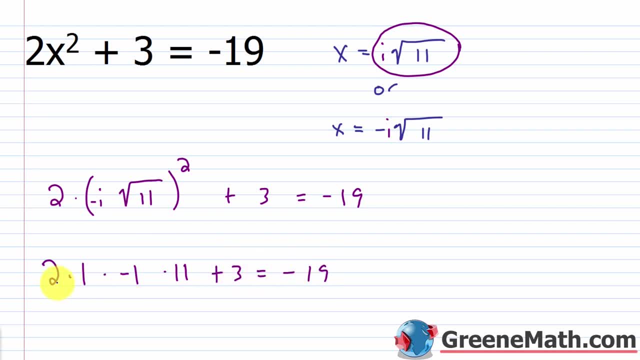 plus 3 equals negative 19.. So 2 times 1 is 2.. 2 times negative, 1 is negative 2.. Negative 2 times 11 is negative 22.. Negative 22 plus 3 is negative 19.. 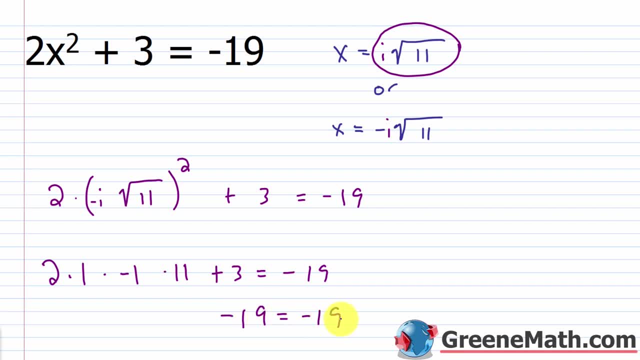 So again you get negative 19 equals negative 19.. So each of these work as a solution. So the solution said you could put negative: i times the square root of 11, comma, i times the square root of 11,. or if you wanted to write this: 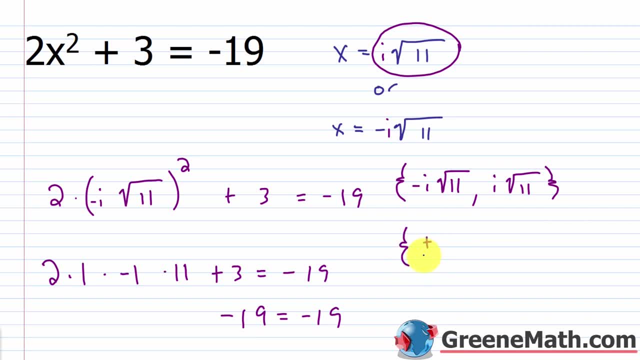 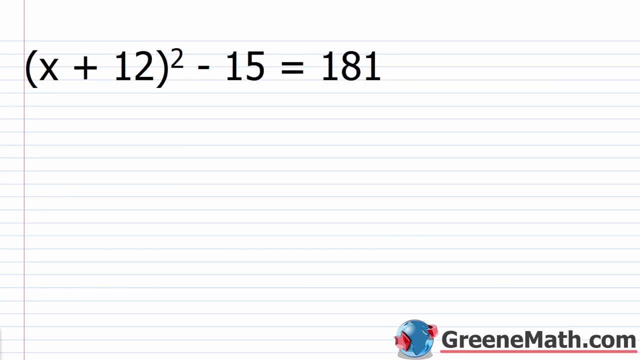 in a more compact format, you could put plus or minus: i times the square root of 11.. All right, let's take a look at something that's a little bit more challenging. So we have the quantity x plus 12, squared minus 15, equals 181.. So can we use our square root? 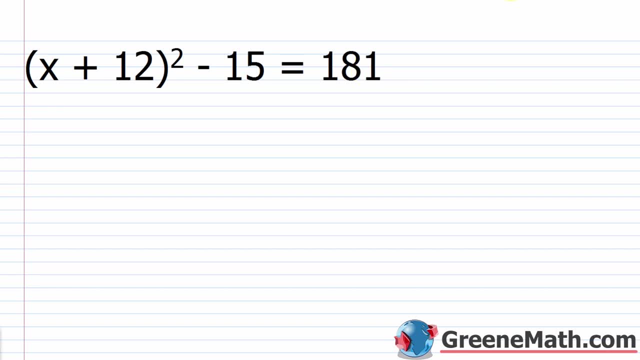 property here. Yes, we can. If this guy right here is squared, that's a perfect square. If I took the square root of it, I'd get x plus 12. So all I need to do for this type of problem is: 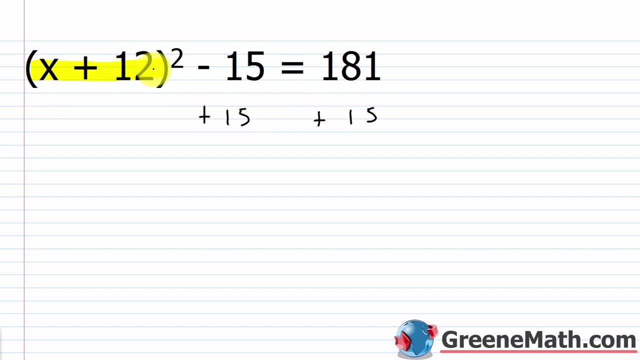 add 15 to each side of the equation so that this guy is isolated. So this would cancel itself out and I would have x plus 12, that quantity squared is equal to 181 plus 15 is going to be 196.. Now all I need to do now is just take the square root of each side. So I'm going to take the. 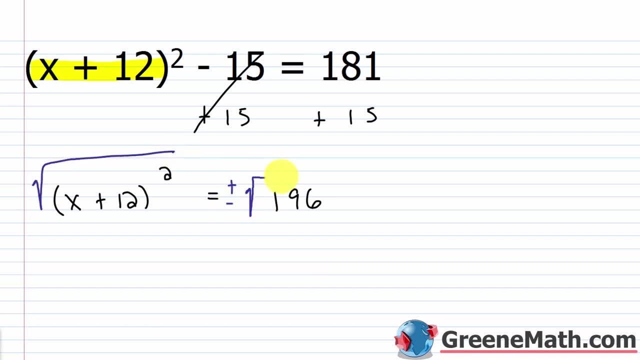 square root of this side, and then I'm going to put plus or minus the square root of this side, So this would cancel with this and I'm going to be left with this x plus 12.. So I'm left with just x plus 12 and this equals plus or minus the square root of. 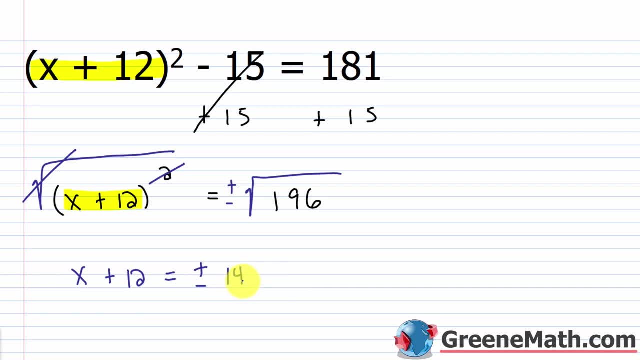 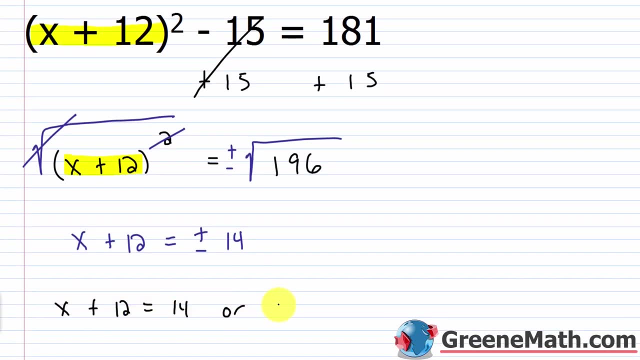 196 is 14, so 14.. So I've got two different scenarios here. I've got: x plus 12 is equal to 14, or x plus 12 is equal to negative 14. And you've got to go through both of those because there's 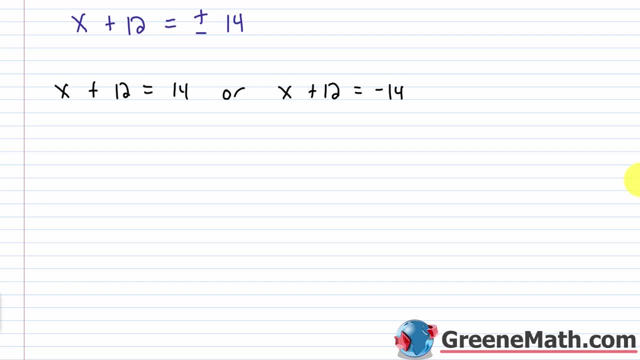 two different solutions. So I'm going to take the square root of this side and I'm going to put 4 over here. All right, now all I've got to do is just save some play here. So I'm going to put x plus 12 and then the square root of this side, So we've got x plus 12. cancel. 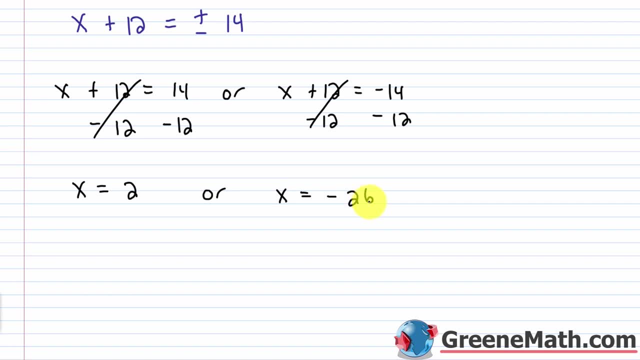 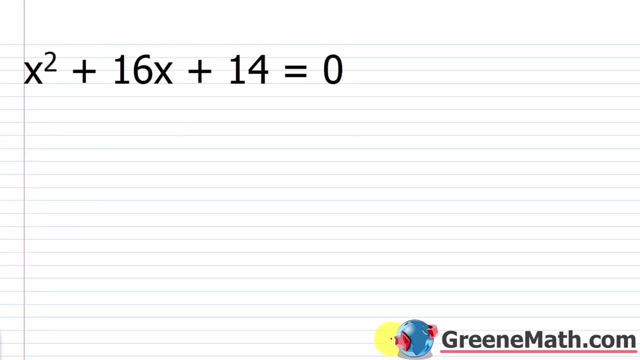 out, And now I can do it any way that I want. So I'm going to make this real quick. All right, and we will have it here at the bottom. here, in this one Lunenberg password team, We are equal to 32, so it's 222.. All right, And if we flip it off, we have 12 over here. 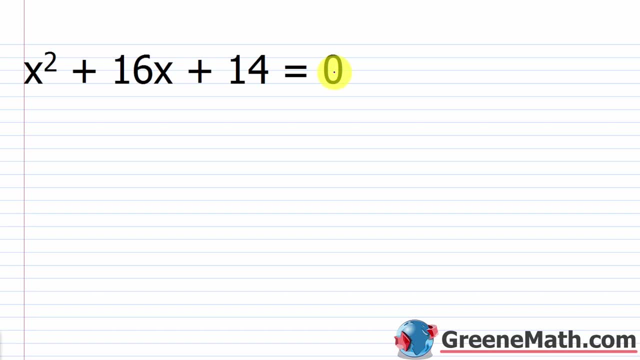 Programmable x times a than 1600. So we have 22.. root property right. some of you will see this and you'll say, okay, we'll just subtract 14 away from each side of the equation, take square root of both sides and we're done. it's not going to work for. 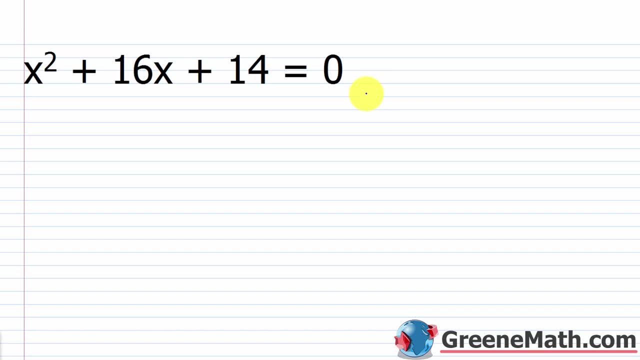 that you need to use a more elaborate process for this, and that process is known as completing the square, and of course you can use the quadratic formula if you want to, but we're not going to get to that till the next lesson. so for completing the square, we'll just go through that real quick. 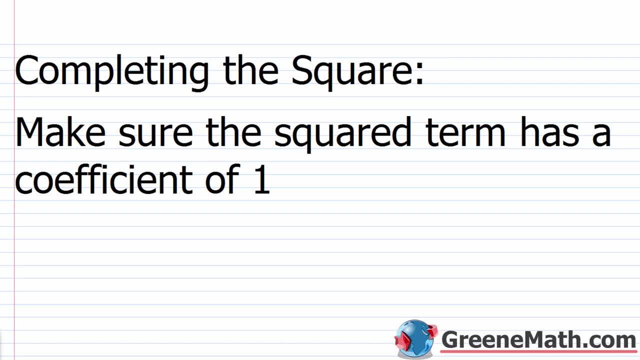 and this is one of those things: you want to write it down and just practice the steps to where they just become second nature for you. it's kind of a tedious process and a lot of students don't like it, but you want to make sure that you memorize it because once you get to using the quadratic, 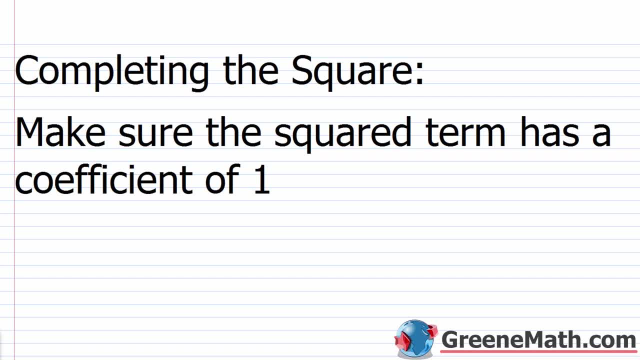 formula. you're not really going to go back to this because of how tedious it is, and then if you need to use it later on, you will have forgotten this process. so the first thing to do is to make sure the square term has a coefficient of one. so if we go back up- and i'll kind of jump back and 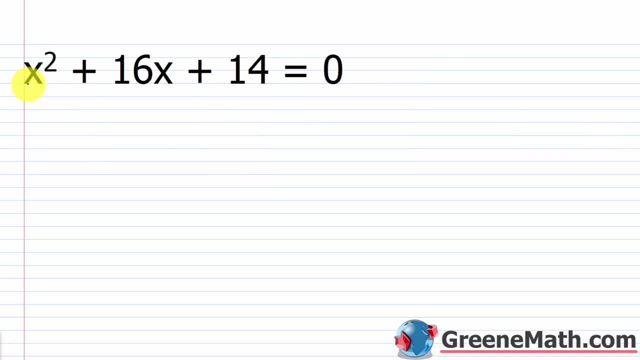 forth. this already has a coefficient of one, so we're good to go there you. the next thing you want to do is you want to move all the variable terms to one side and the constant to the other. so for this one i could just subtract 14 away from each side of the. 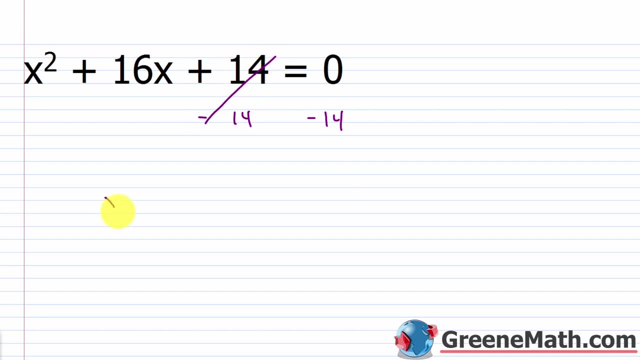 equation. this would cancel. we would have x squared plus 16x, and then i'll move this kind of down because we're going to put something in that place right there. this will be equal to negative 14. so all the variable terms are on one side. these are the variable terms. 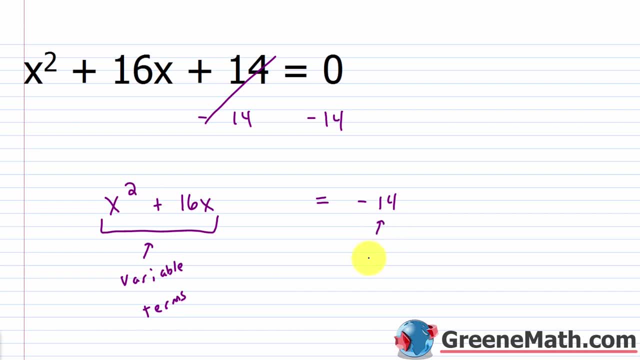 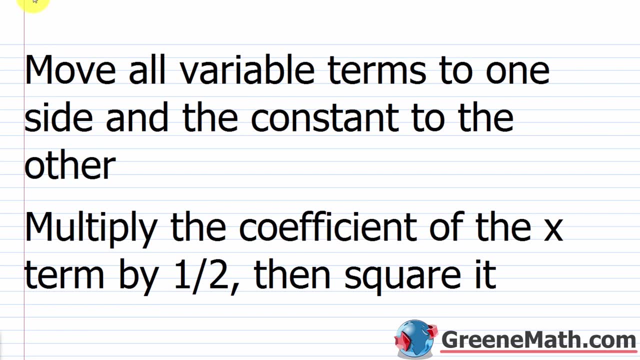 and the constant is on another side. by itself, this is your constant. all right, the next step is the one that's the most confusing. you want to multiply the coefficient of the x term- just the coefficient- by one half, then square it, so here's the coefficient for. 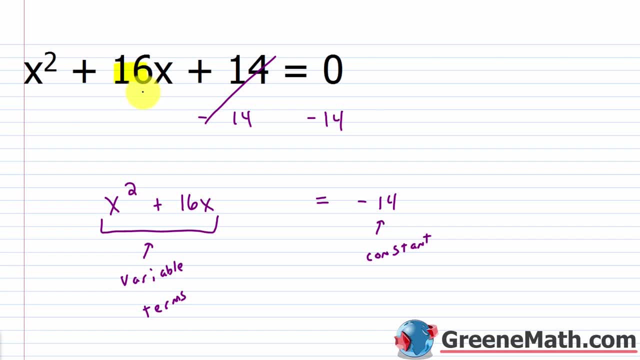 the x to the first power term, it's a 16.. if i multiply 16 by one half and then i square it, what am i going to get? 16 times a half is 8, 8 squared is 64.. now you're going to use this. 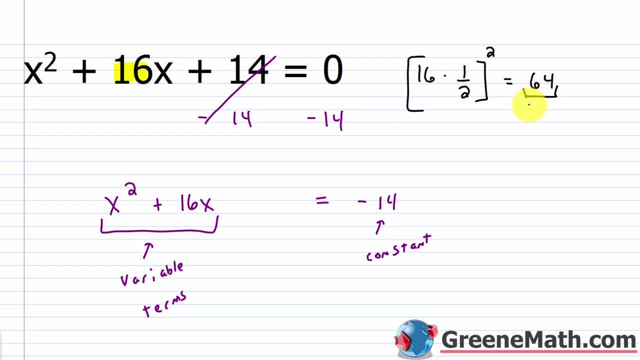 in one second. i just want to relay a simple trick to remembering this step. when i was in high school, i struggled with remembering this. i didn't practice the steps like i should have, and one day our teacher said something to it. she said: caught it in half and square it. caught it in half. 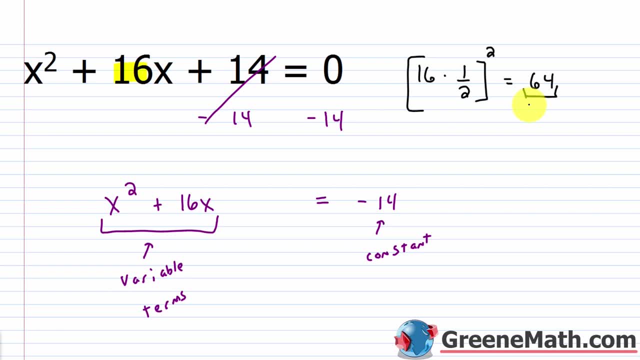 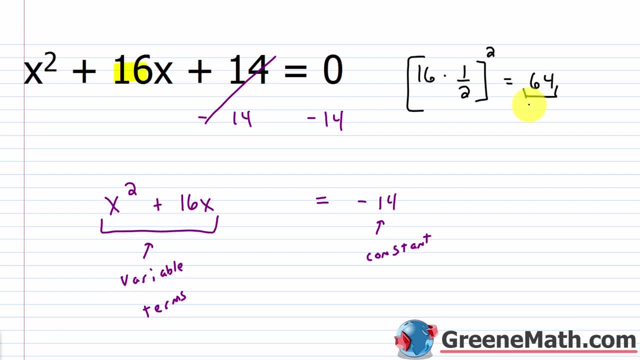 easy to remember. So cut it in half and then square it. Okay. so that's what we've done here. We've cut the number 16 in half, by multiplying by a half, That gave us 8, and then we squared it to. 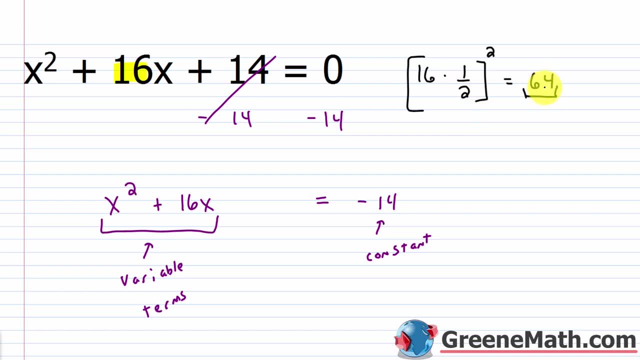 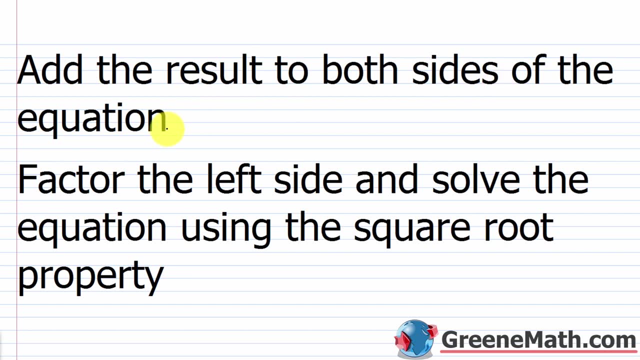 get 64. Now, what do we do with 64?? Well, what we do is we add the result- which again, in this case, is 64, to both sides of the equation. Now, when we do that, let me just go back up real quick. 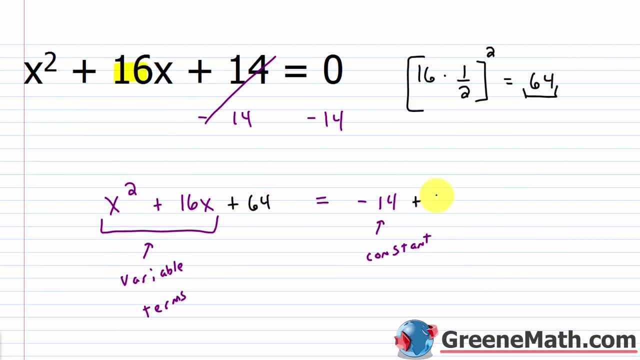 what's going to happen is the left side of the equation is now a perfect square trinomial. Some of you know what that is. Some of you are like: what is this guy talking about? What is a perfect square trinomial? So, as a little side note, let's just show you what that is real fast. 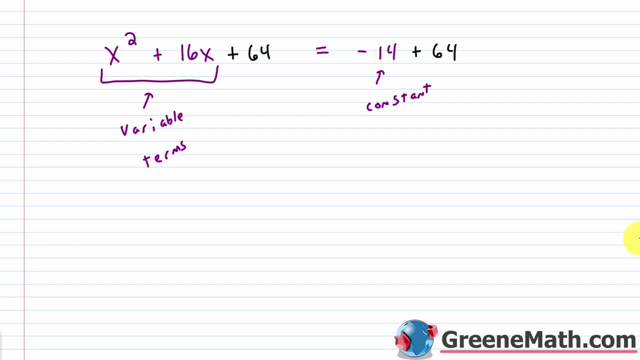 We talked about special products and special factoring a lot. If you have something like x squared plus 2xy plus y squared, this is x plus y. that quantity squared, All a perfect square trinomial is, is something that you could take that looks like this: 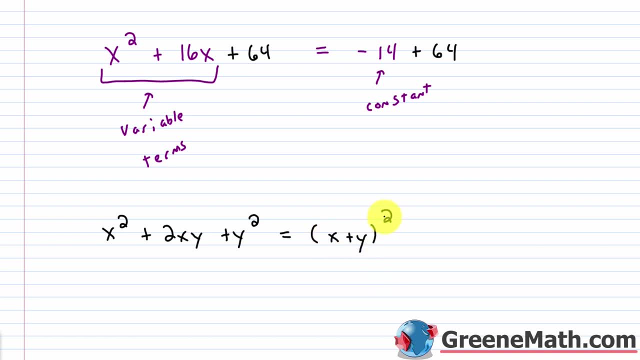 and you could factor it into a binomial squared. That's all it is Completing. the square just gives you one side of your equation as a perfect square trinomial, which allows you to factor it into a binomial squared, which then allows you to use the square root property. 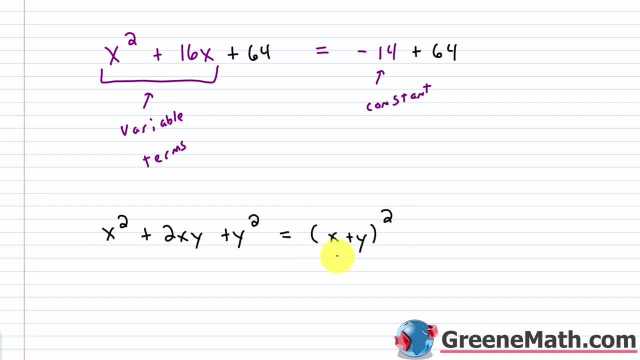 Because I could just take the square root of this guy and I'll just have what's in parentheses For this guy right here, this x squared plus 16x, plus 64, again, if I think about special factoring, I know that this guy goes here right, So just x goes there. And then this guy: 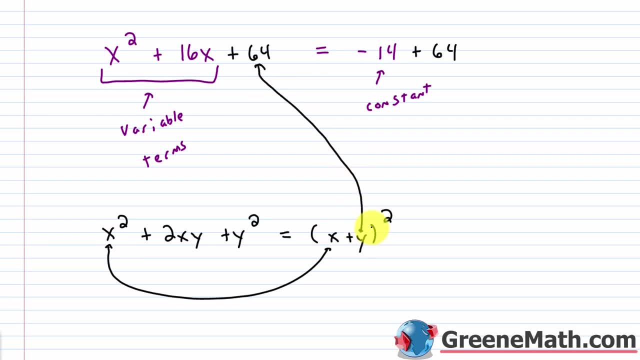 the square root of that would go here. So all I need to think about is: what is the square root of x squared? That's x, And then plus. what is the square root of 64?? That's 8, and that's square. So I've factored my left side and I've got the square root of x squared, and that's 8.. And then I've got the square root of x squared, and that's 8.. And then I've got the square root of x squared. 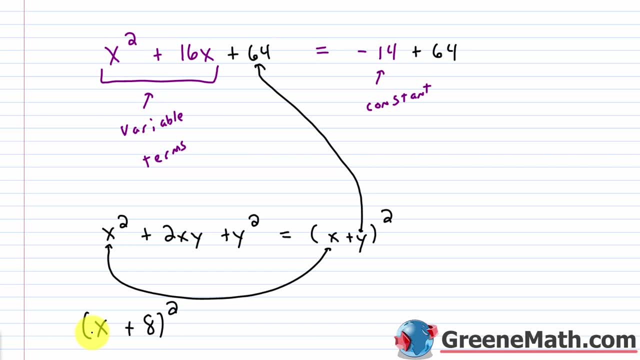 into the quantity x plus 8 squared. Now let me erase this real quick. I'm going to just drag it up And this is equal to over here. I just need to do a sum Negative: 14 plus 64 is going. 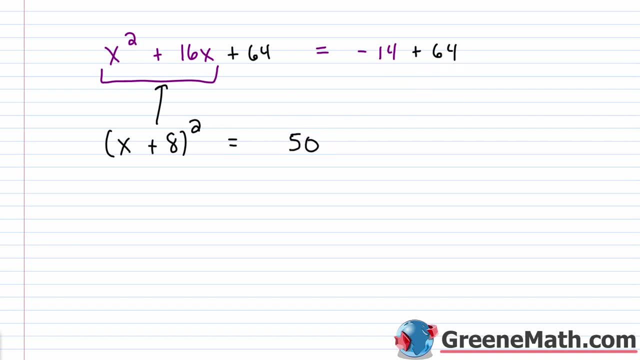 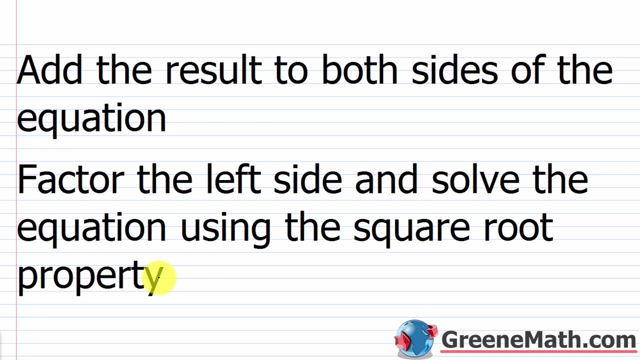 to give me positive 50.. Now let's go back down And again factor the left side and solve the equation using the square root property. Okay, solve the equation using the square root property. So we've already factored the left side. So all we need to do is take the square root of this side. 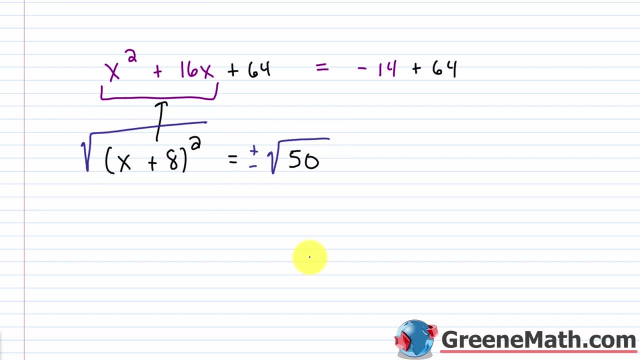 and then put plus or minus the square root of this side. So this will cancel with this And we just have x plus 8. And this is equal to plus or minus the square root of 50.. Now this is where it gets even more tedious, because the square root of 50, 50- is not a perfect square. So we've got. 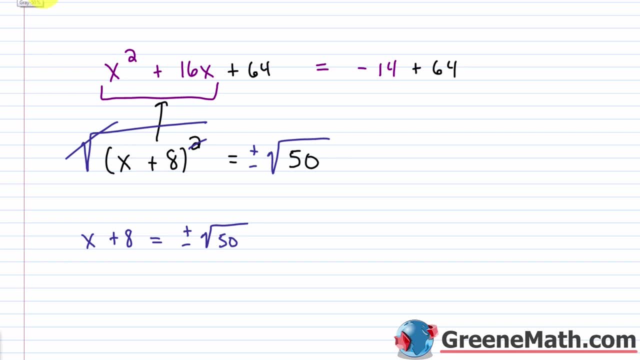 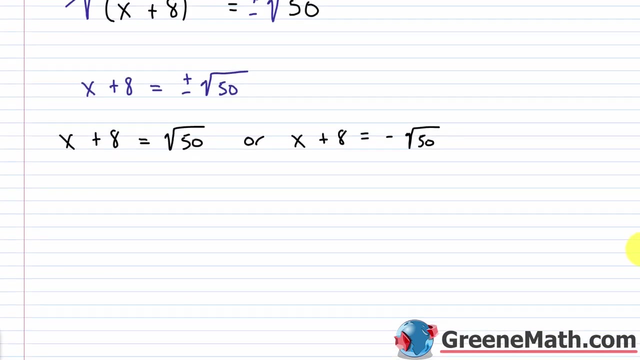 to think about how to simplify that. Let's just start out by saying that this is: x plus 8 is equal to the principal square root of 50, or x plus 8 is equal to the principal square root of 50, plus 8 is equal to the negative square root of 50.. Let's scroll down a little bit. So the square root. 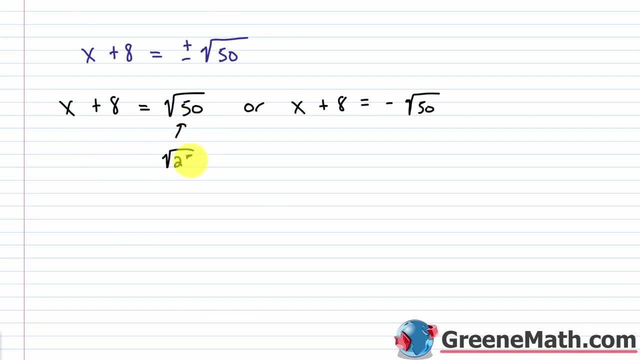 of 50 is what It's: the square root of 25 times the square root of 2.. Square root of 25 is 5.. So it's basically 5 times the square root of 2.. This is 5 times the square root of 2.. This guy right. 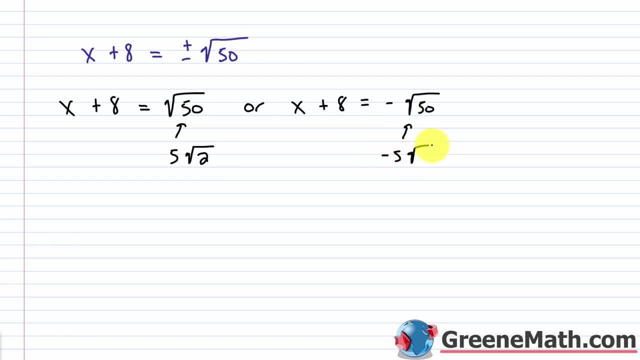 here- I might as well say it's negative- 5 times the square root of 2.. And so what do we have here? You would have: x plus 8, is equal to 5 times the square root of 2.. We could subtract 8 away from each side of the equation. 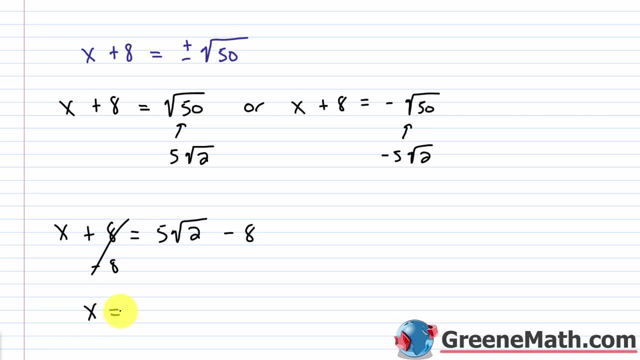 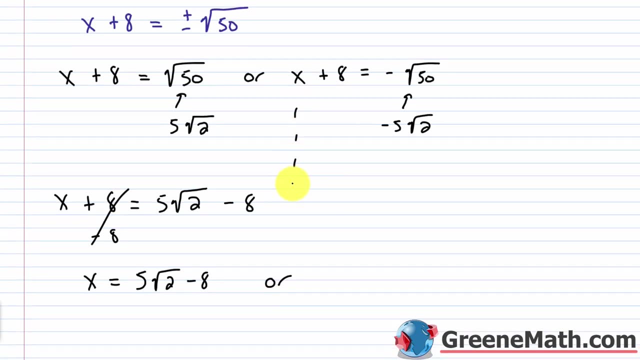 That would go away And you'd simply be left with: x is equal to 5 times the square root of 2 minus 8.. Then, or over here, I would have: x plus 8 is equal to negative 5 times the square root of 2.. 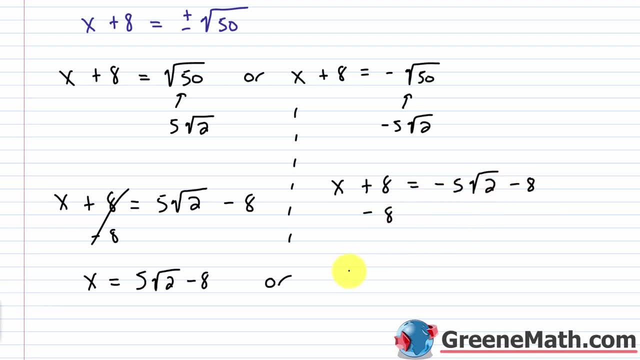 We would subtract 8 away from each side of this equation And we'd end up with x is equal to negative 5.. Now, if you wanted to write this more compactly, what you could do? you could say that x is equal to. 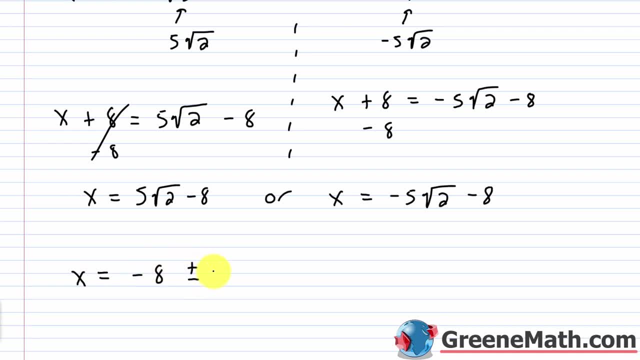 negative 8 plus or minus 5 times the square root of 2.. So this accounts for 5 times the square root of 2, and it accounts for negative 5 times the square root of 2.. So in solution set notation: 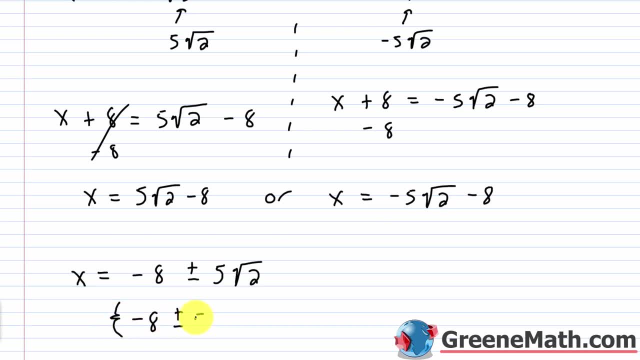 we'll say negative, 8 plus or minus 5 times the square root of 2.. Now you're free to check each solution set notation. We'll say negative, 8 plus or minus 5 times the square root of 2.. I've already checked them. I know they work. It'd be good practice for you to do it In the 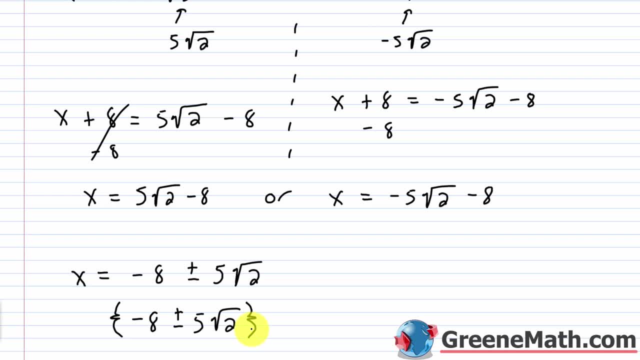 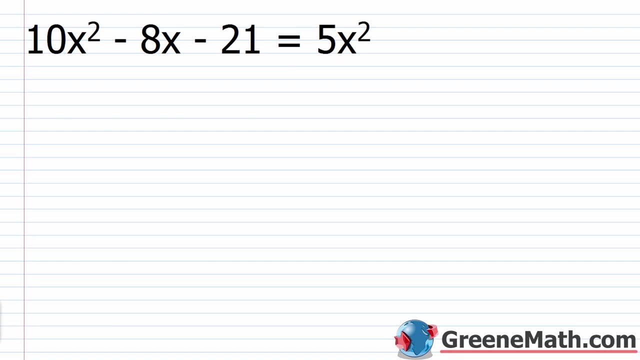 interest of time and making this video a little bit shorter, I want to just stop right here and move on to the next problem. All right, So let's take a look at another one. So we have 10x squared minus 8x minus 21 equals 5x squared. So the first thing we're going to do, we're going to have this. 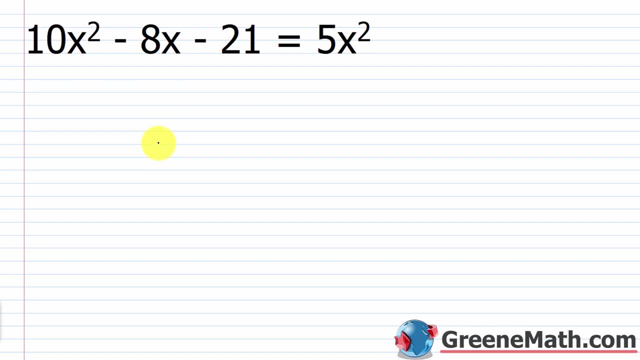 in the format of ax squared plus bx plus c equals 0.. So let's just subtract 5x squared away from each side of the equation. That's going to cancel and become 0, and this is equal to 10x squared minus 5x squared is 5x. 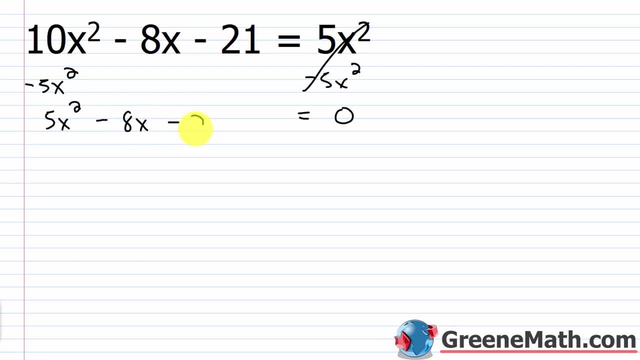 squared, And this is minus 8x, minus 21.. Again, it equals 0.. Now, in this particular case, the coefficient for x squared is not 1.. You have a 5 hanging out there. You don't want that. 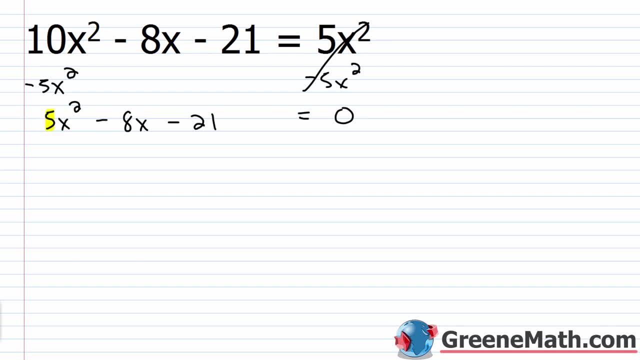 okay. So what you're going to do is you're going to divide both sides of the equation by 5.. So I'm going to divide this by 5, this by 5, this by 5, and this by 5.. 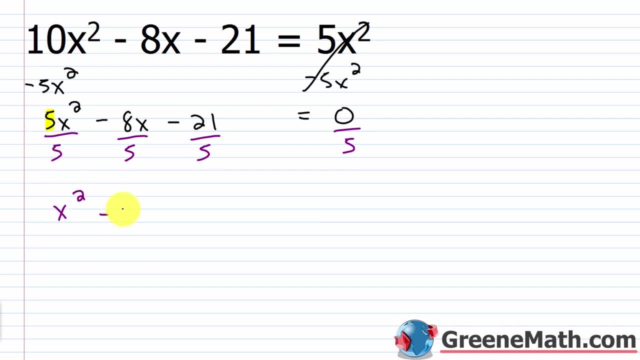 So we know that this would give me x squared minus 8 fifths. x minus 21 fifths is equal to 0. divided by 5 is just 0.. Now the next thing that I want to do, I want to move all my variable terms. 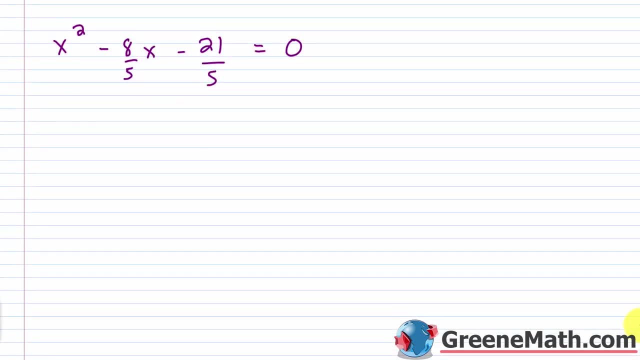 to one side, all my numbers to the other. So I'm simply going to add 21 fifths to both sides of the equation, So you'll have x squared minus 8x squared minus 21 fifths is equal to 0.. And I'm going to 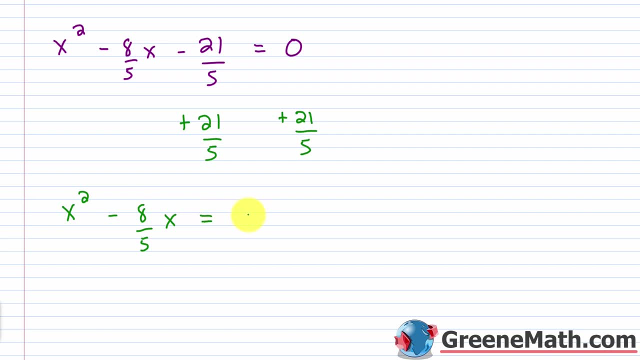 take this coefficient for the x to the first power variable, I want to cut it in half, meaning multiply by half and then square it. I'm going to take that result and add it to both sides of the equation. So over here. if I did that, if I had negative 8 fifths and I multiply by half. 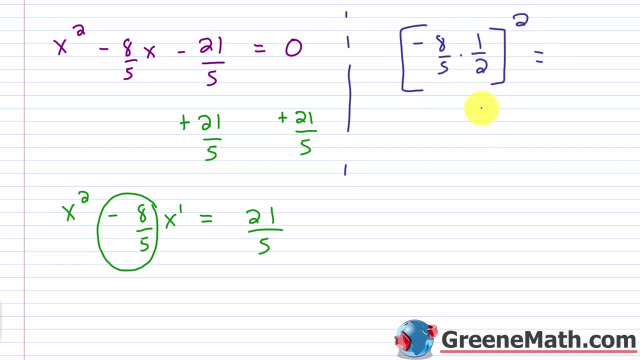 and then I square this. what am I going to get? Well, this would cancel with this and give me, so it would be negative. 4 fifths squared. The negative square would be positive. So don't worry about that: 4 squared is 16,, 5 squared is 25.. So what are we going to have? Let's kind of. 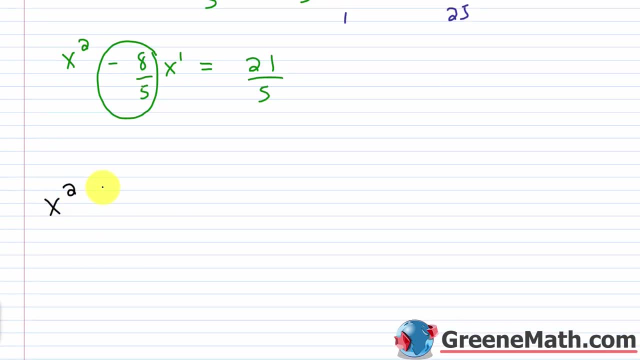 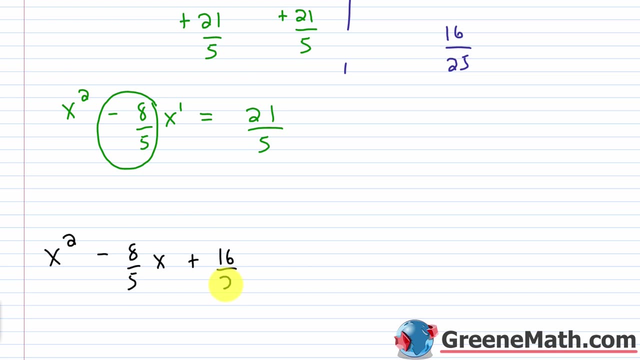 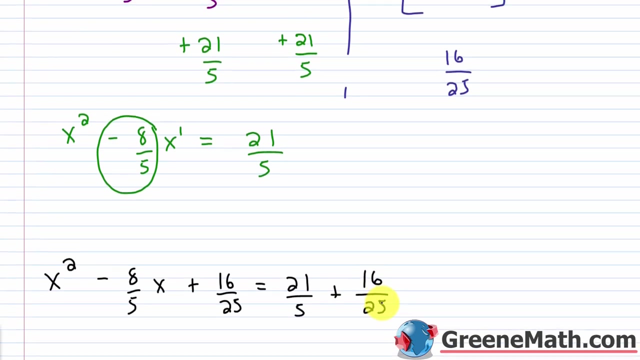 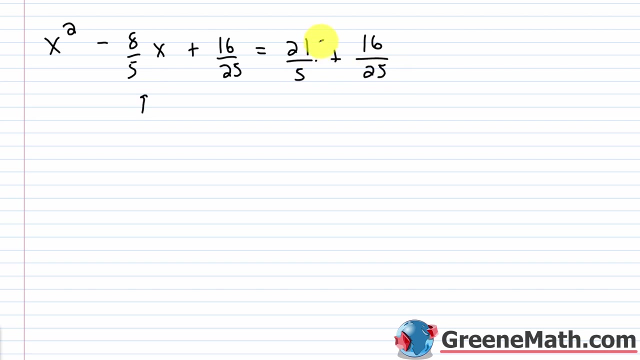 scroll down. We're going to have x squared minus 8 fifths x, and then plus 16 twenty-fifths. This equals 21 over 5 plus 16 twenty-fifths. This left side is a perfect square trinomial. The right side is just going to be a constant. I just need to multiply this by 5 over. 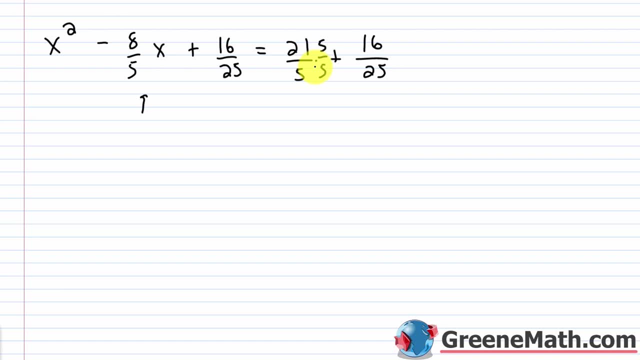 5.. So I have a common denominator and I can figure out what this side is going to be. So 21 times 5 is 105.. If we add 105 and 16, we get 121. So this is 121 over 25.. Now on the left side. 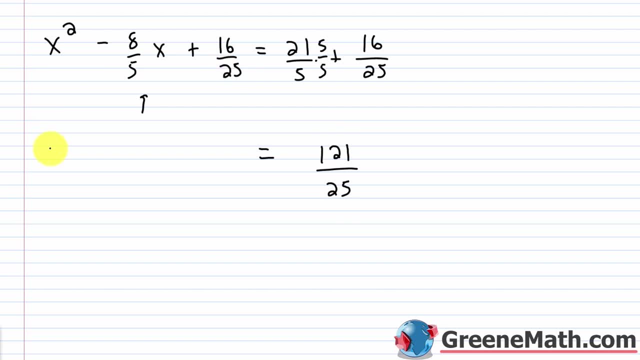 again, this is a perfect square trinomial that we've created, So following the pattern from special factoring. I know it's something. In this case you have a minus, So minus something else, That quantity is squared. It's always the square root of this guy. So the square root of x squared is x. 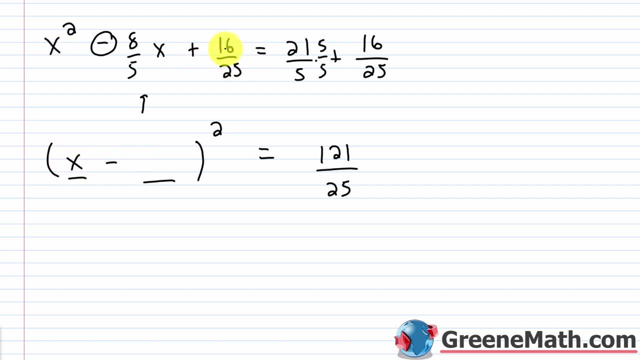 And then the square root of this guy, the square root of 16 over 25.. Well, we know, if we take the square root of 16 over 25, we get 4 fifths. So 4 fifths goes there. 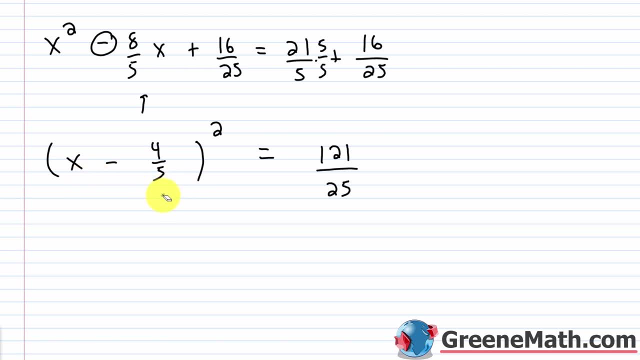 So we've got x minus 4 fifths. That quantity squared is equal to 121 over 25.. And then now I could take the square root of each side. So I'll take the square root of this side And then plus or minus the square root of this side, So what we'll have- x minus 4 fifths is equal. 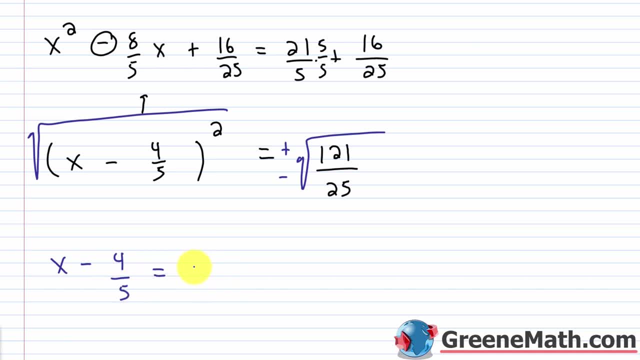 to: you've got the principal square root of 121 over 25,, which is 11 fifths, And you'll say: or you've got x minus 4 fifths is equal to the negative square root of 121 over 25.. 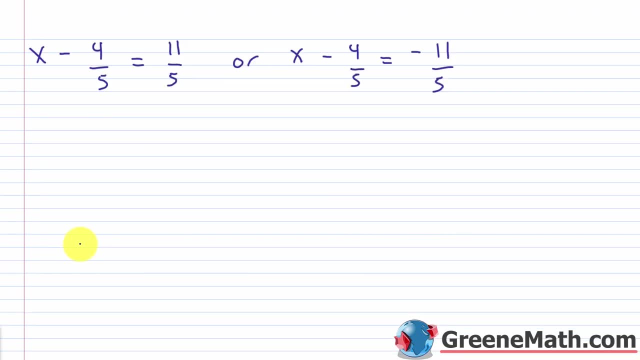 So that's negative 11 fifths. All right, So now let's solve these two equations. If we add 4 fifths to To each side over here, what are we going to have? You'll have: x is equal to 11 plus 4 over. 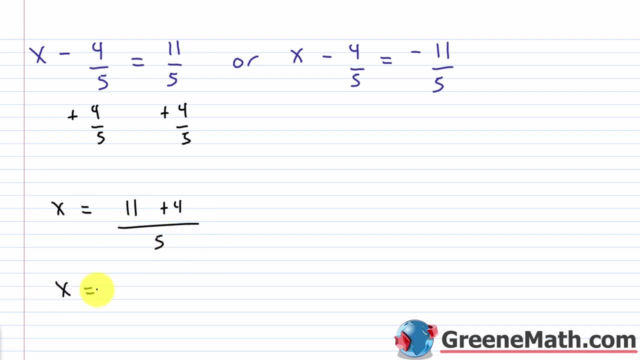 that common denominator of 5.. So you'll say x is equal to 15 over 5,, which is 3.. Then over here you'll have 4 fifths added to each side of the equation. So we'll have: x is equal to negative 11 plus 4 over the common denominator of 5.. 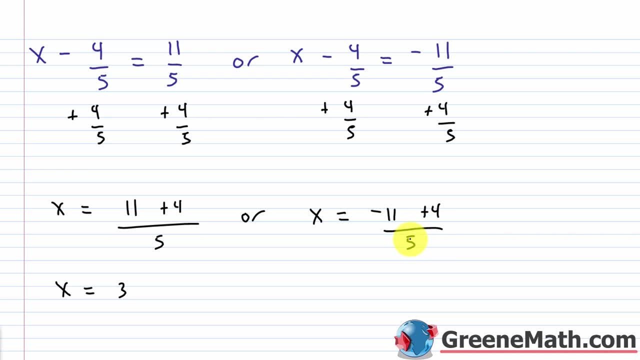 11 plus 4 is negative 7.. Negative 7 over 5 is negative 7 fifths. So x equals 3 or x is equal to negative 7 fifths. So in solution set notation we'll go ahead and say this is negative 7 fifths. 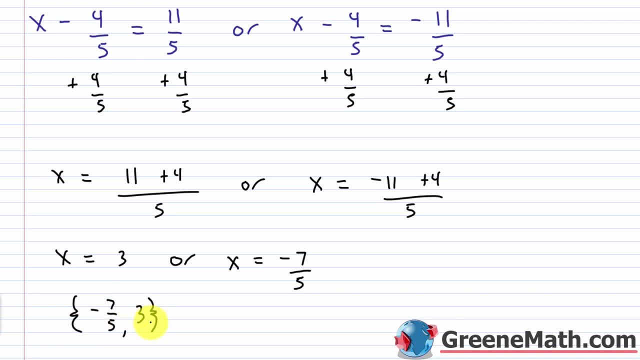 comma 3.. And again, if you want to check these, go back and plug negative 7 fifths in for x in the original equation. Verify the left and the right side are equal. Then plug 3 into the original equation for x. 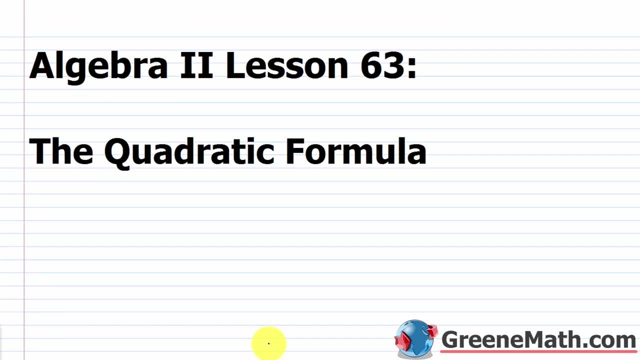 Verify: the left and the right side are equal. Hello and welcome to Algebra 2, Lesson 63. In this video we're going to learn about the quadratic formula. So for the majority of you that did take an Algebra 1 course, you remember the quadratic. 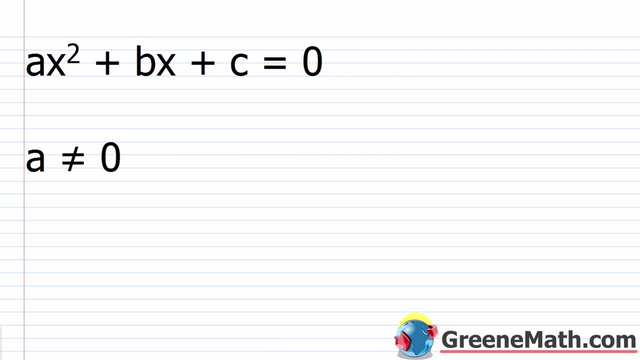 formula. It's generally going to be the final thing that you learn in Algebra 1 before you kind of take your break and you come back the following year and you start Algebra 2.. Or in some cases you might start Geometry, just depending on where you live. 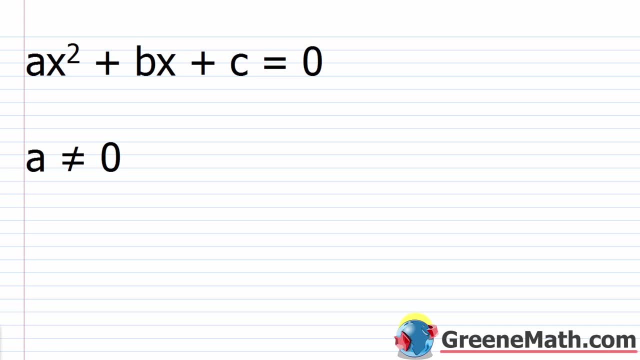 But for the course we're going to learn about the quadratic formula. So for the course we're going to learn about the quadratic formula. So for the course we're going to learn about the quadratic formula. A lot of you will find that it's kind of a relief, right? Because when you work with 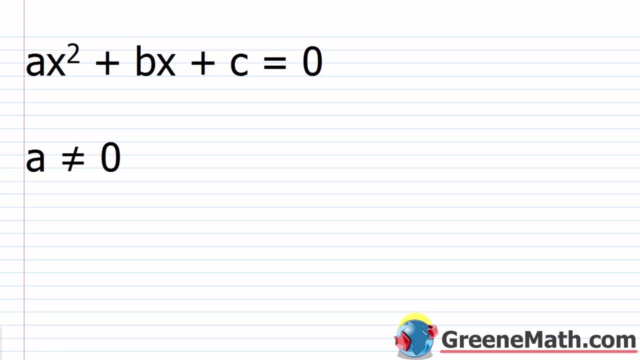 quadratic equations. there's kind of two different scenarios. There's kind of the less tedious ones that you can solve using factoring, And then there are the more tedious ones, to where you can't solve it using factoring. So you've got to use this kind of messy and tedious completing the square method. 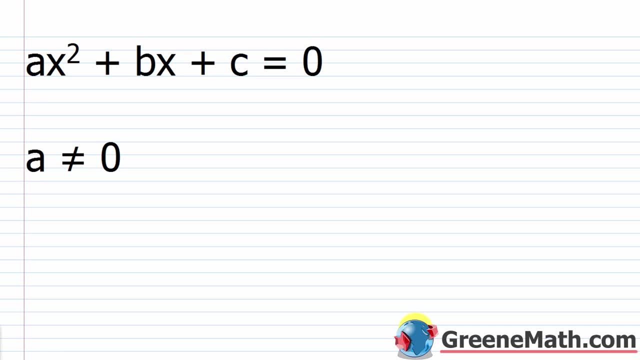 So a lot of us don't like using it. I personally don't like using it. I don't know anybody likes using it- But it's something that you can do, And I'm going to show you how to do it. So let's go. 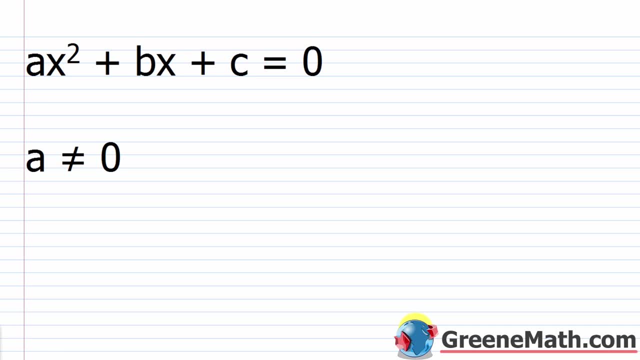 ahead and start Algebra 2, Lesson 63. But it's something that is necessary to learn because you will be tested on that at some point in your life. But, moving kind of forward, you don't need to rely on either of those. You don't. 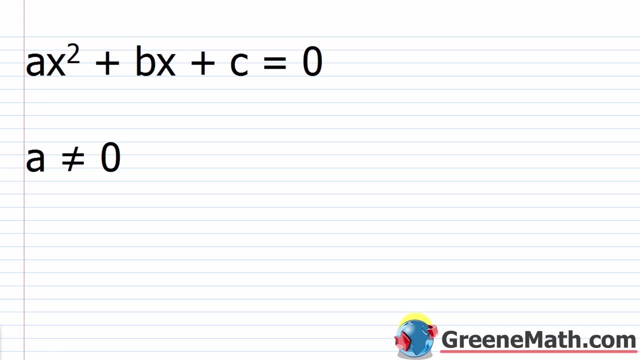 have to factor things anymore. You don't have to use completing the square because there's a catch-all method known as the quadratic formula. So with a quadratic formula we just take this generic ax squared plus bx plus c equals zero Again, where a, b and c are real numbers. 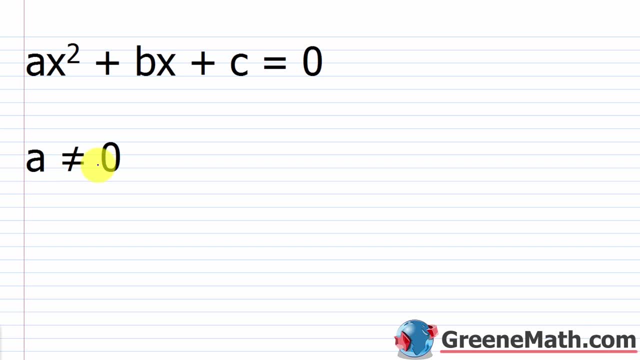 and a is not allowed to be zero, And we just solve it using completing the square. So it's done for us to where we can just plug in for a, b and c, And then we just simplify and we have our solution. 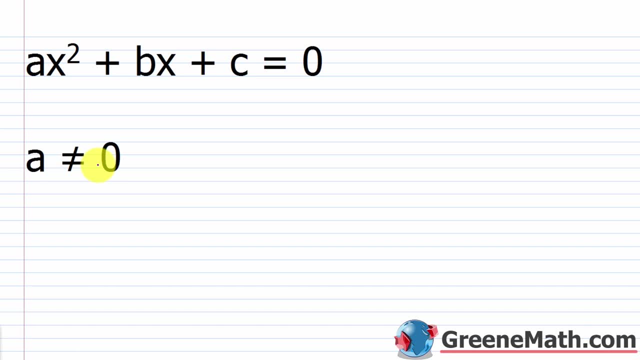 So I want to take you through that real quick. You might never have to derive the quadratic formula in your class, but you also might get in a situation where you do have to derive it. So let's start out with: ax squared plus bx plus c is equal to zero. 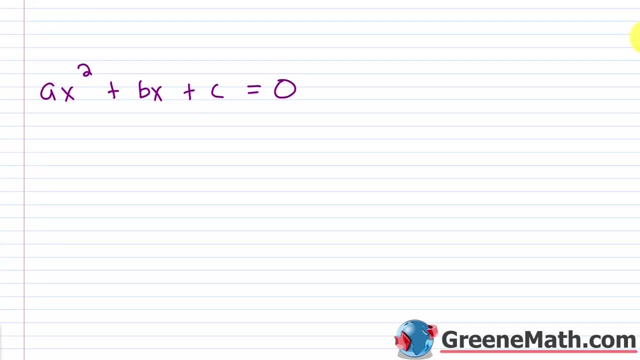 So how would I complete the square if I had that? Just pretend like you had numbers for a, b and c. What would you do? Well, you want to start by making sure that this guy right here is a one. Right now it's an a, so I don't know what it is. All I know is it's not allowed to be zero. 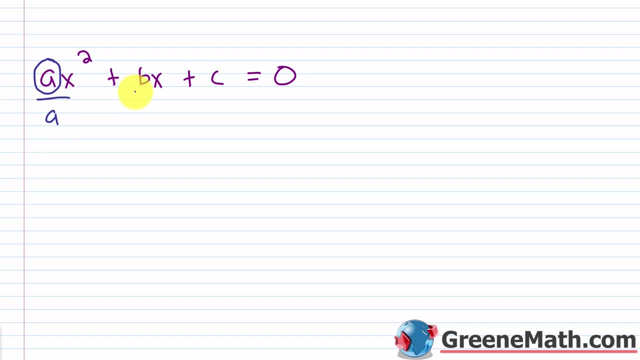 But to make sure that it's a one, I can divide both sides of the equation by a. So a divided by a is one. So now I just have x squared, then plus b over c, And then I can divide both sides of the equation by a. 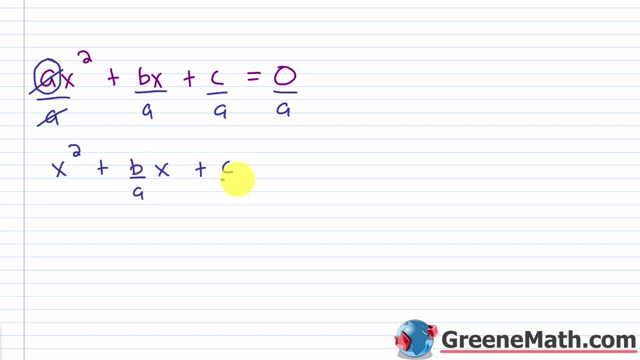 So b over a times x plus c over a, and this would be equal to zero over a, which is zero. Now what's the next step? We want to make sure all the variable terms are on one side and then all the numbers are on the other, So we want these guys right here on one side. 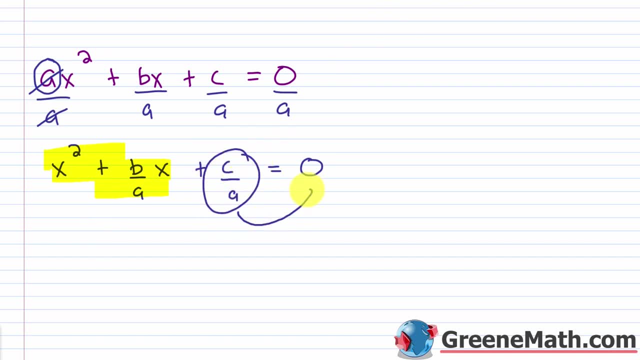 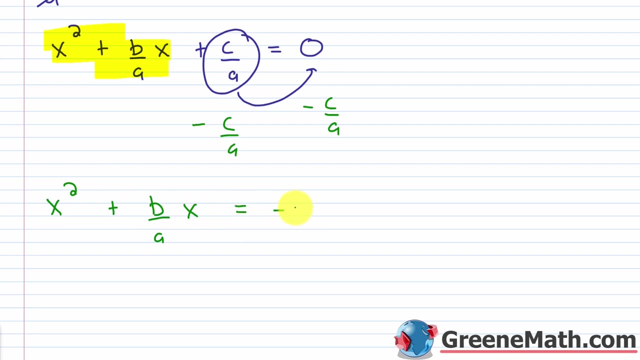 and then we want this guy on the other side. So let's move this over here. So let's subtract c over a, away from each side of the equation, So that's going to give us x squared plus b over a times x. This will be equal to negative c over a. 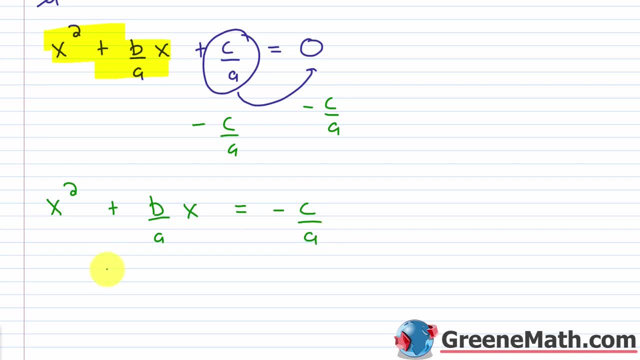 The next step is to complete the square, meaning we want the left side to turn out to be a perfect square trinomial. So to do this, again we look at the coefficient for our variable raised to the first power. So in this case that coefficient is b over a. 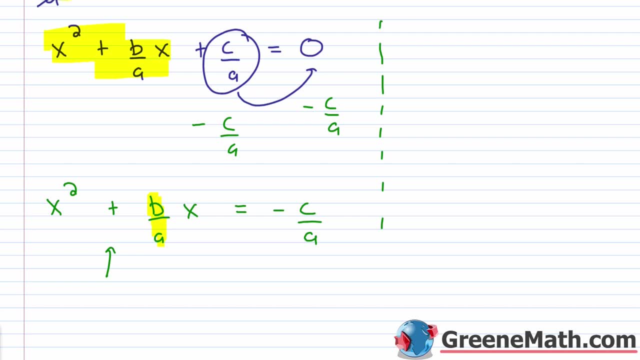 We want to cut it in half, or again multiply it by a half, So b over a multiplied by a half. And then we want to cut it in half, or again multiply it by a half, So b over a multiplied by a half. 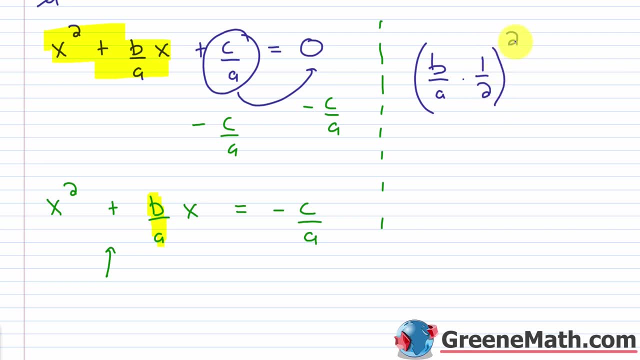 And then we want to square the result, And I always say: cut it in half and then square it. So what will we get here? You get b over 2a, and that would be squared. Remember, everything here has to be squared. So b is going to be squared over 2, which is squared, which is: 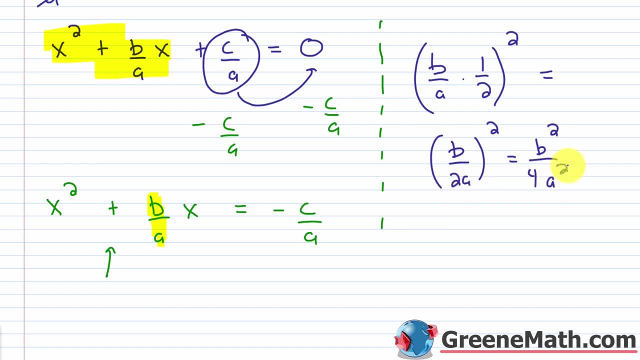 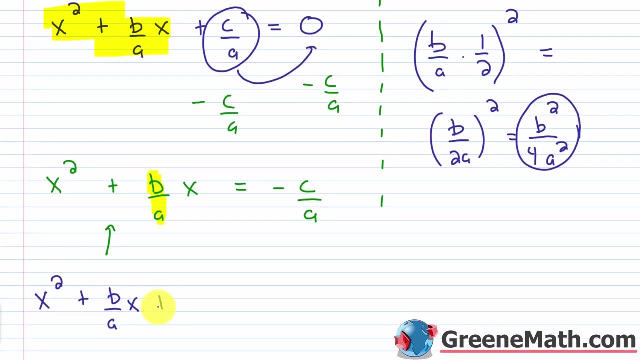 4. And then a is squared, that's a squared. So what I'm going to do is I'm going to add this to both sides of the equation so that the left side is a perfect square trinomial. So we will have x squared plus b over ax plus b squared over 4a squared, This is equal to: 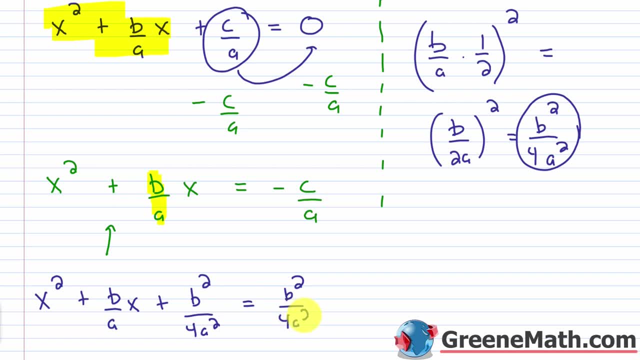 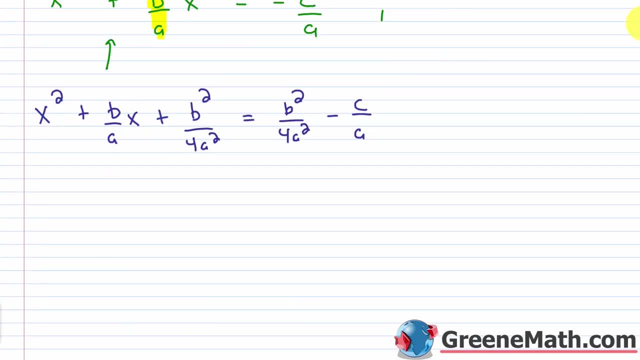 b squared over 4a squared minus c over a. All right, let's scroll down and get a little room going. Now, what do I want to do next? Well, I know that this is a perfect square. trinomial: This is a perfect square. 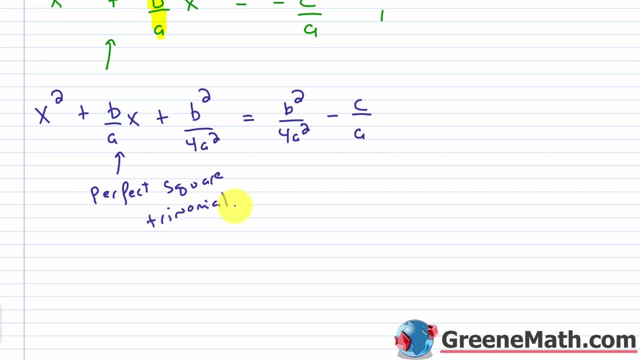 Trinomial. What does that mean? in case you don't know, It means that I can factor this into the product of a binomial squared. So something plus something squared would get me that. Now, if you remember from your special factoring in your special products lessons. 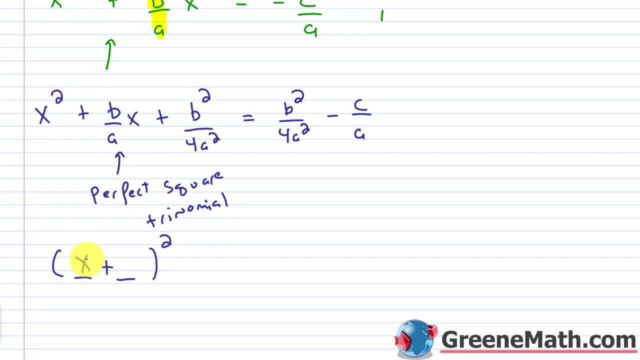 this would be what. I would take this as x squared, so this would be x, And this is b squared over 4a squared. We just figured out what this was, because we squared this to get to this, So it's just b over 2a. So then, right here, I'm going to have b over. 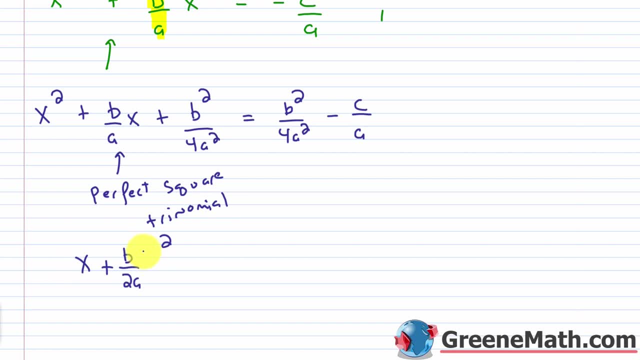 kind of erase these 2a. So this is equal to: we have b squared over 4a squared minus. if I wanted to get a common denominator going, I would multiply this by 4a over 4a, So 4a. 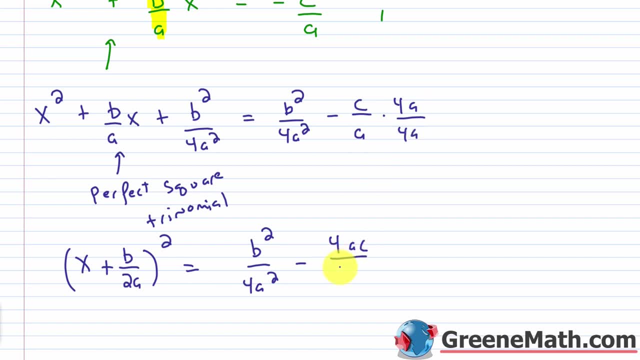 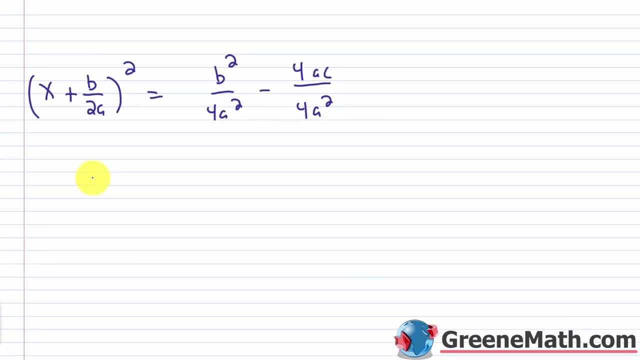 times c would be 4ac, then 4a times a will be 4a squared. So let's copy this. I'll bring it down And just continuing. So this guy on the left is x plus b over 2a. Again, this is squared. This equals We have a. 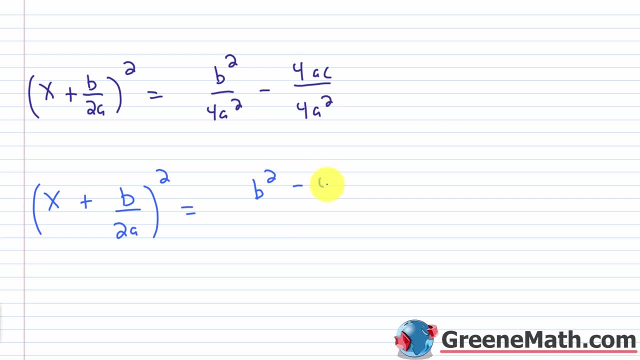 common denominator now. So we can write b squared minus 4ac over the common denominator of 4a squared. So what I want to do now is I want to use my square root property. I'm going to take the square root of this side And I'm going to say: this is plus or minus the square root of this. 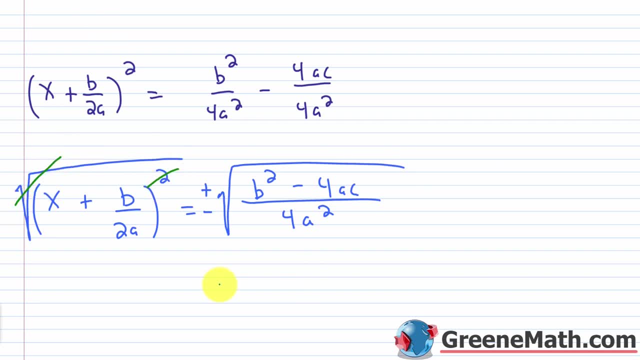 side. So this will cancel. with this We'll have x plus b over 2a And this is equal to. let me scroll down, get a little room going. We'll have plus or minus. You have, and I'm just going to. 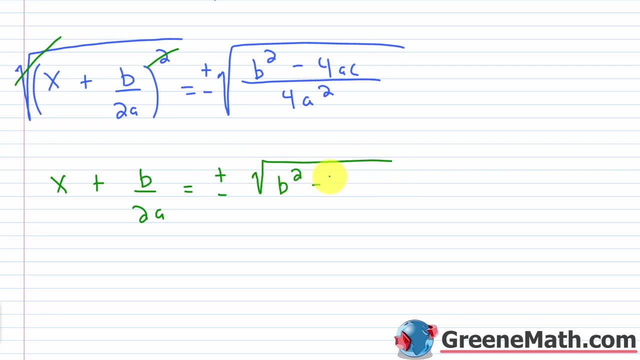 break this up: the square root of b squared minus 4a squared And this is equal to- let me scroll down, get a little room going- We'll have plus or minus b squared minus 4ac over the square root of 4a squared. Let's just write the square root of 4a squared Now. 4a squared is a perfect. 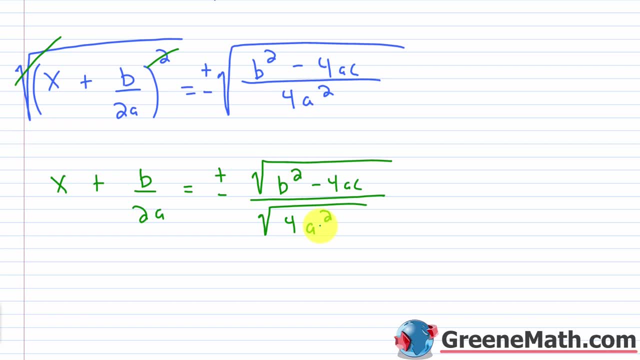 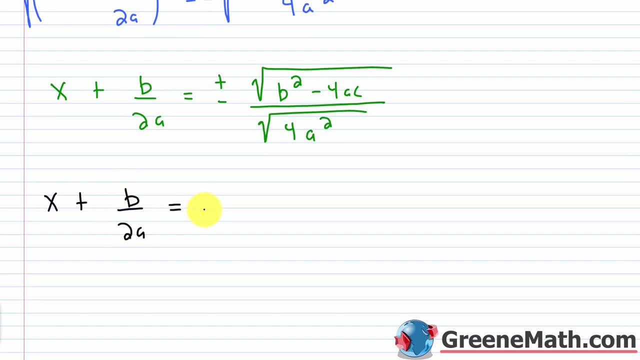 square. Square root of 4 is 2.. Square root of a squared is a. So let's keep simplifying. This will be x plus b over 2a, which is equal to plus or minus the square root of b squared minus 4ac. 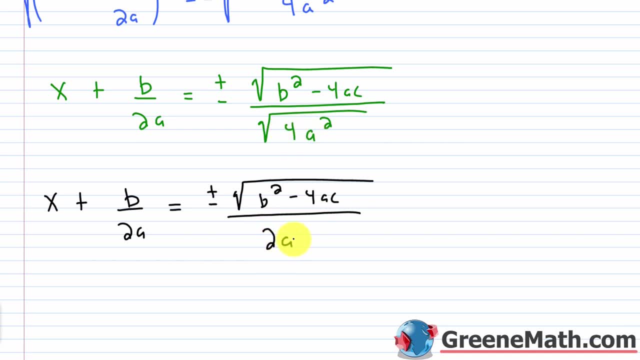 over again. the square root of 4ac, Square root of 4a squared is 2a. Now the next thing I want to do, let me subtract b over 2a, away from each side of the equation, And let's scroll down. get a little room going, So what? 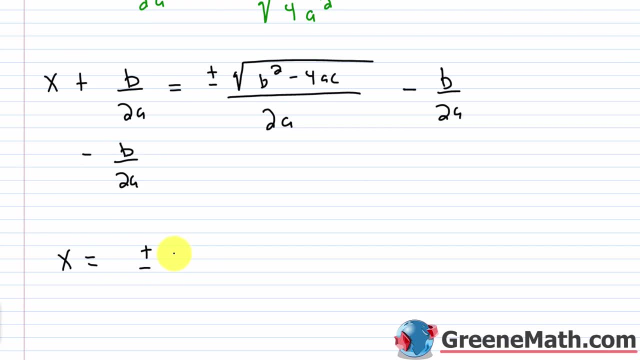 we're going to have is: x is equal to plus or minus, the square root of b squared minus 4ac, then minus b. this whole thing is over 2a. Now the quadratic formula is here. It's just not usually written like this. It's just a square root of b squared minus 4ac over 2a. So let's. 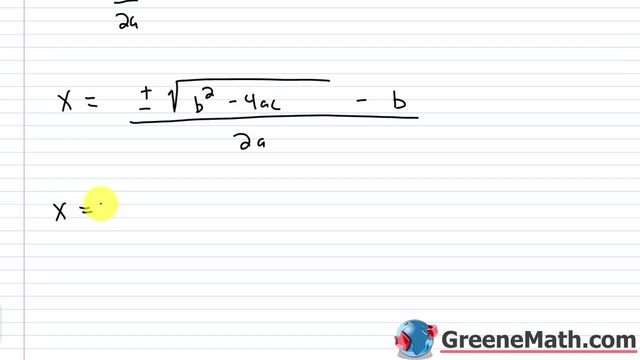 do this. There's one more step to do. So we have x is equal to. I'm going to take this negative b and put it all the way at the far left. So I'm going to put minus b or negative b, then plus or 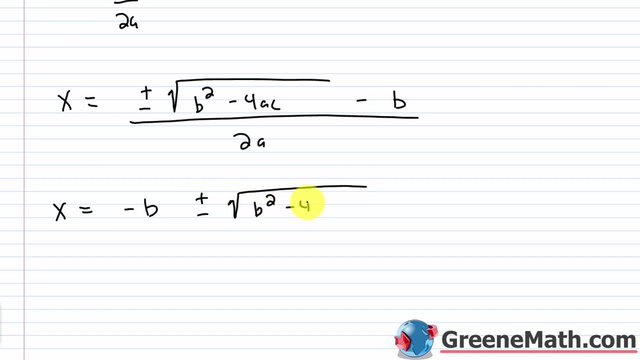 minus the square root of b squared minus 4ac, And then this whole thing is over that denominator of 2a. So this is the quadratic formula. This is the quadratic formula. Now all I need to do is write the square root of b, squared minus 4ac over 2a over 2a. So I'm going to. 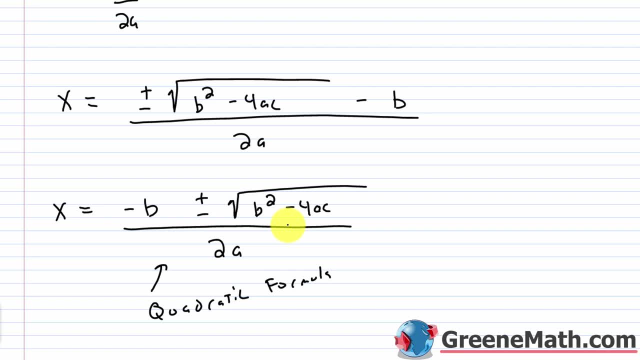 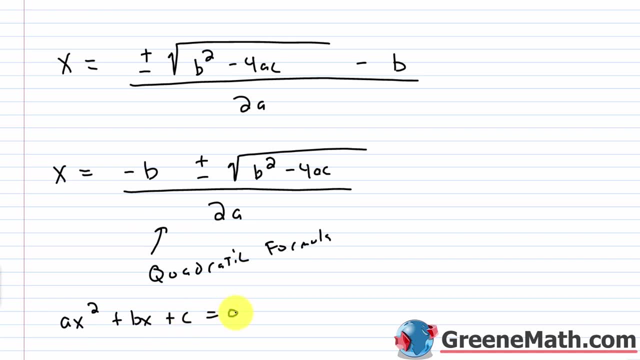 need to do to use this is have my quadratic equation written in standard form, So ax squared plus bx plus c equals zero, And then I just plug in for a, b and c And that'll give me the solutions. Now this part right here: this b squared minus 4ac. this is called the discriminant. 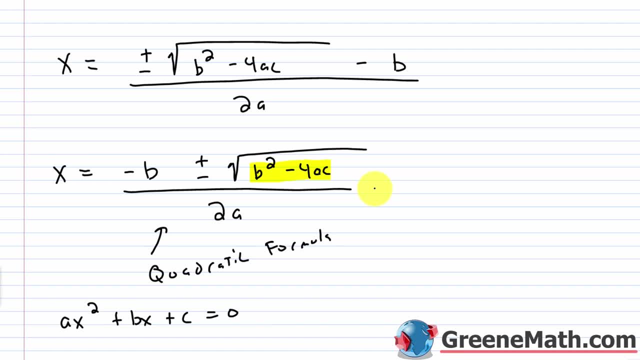 Now the discriminant is going to tell you whether you have a real solution or whether you have a negative solution. So this is going to involve the imaginary unit, right, If you have a negative square root. It's also going to tell you if you have two solutions or just one, If this guy right. 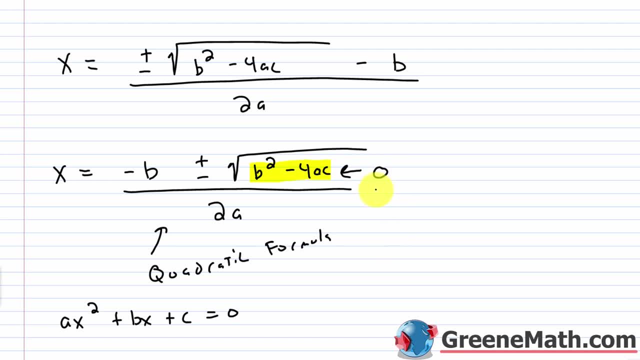 here ends up being zero, you're just going to have one solution, right, Because this plus or minus, plus or minus zero is nothing, right? If you add zero or you subtract away zero, you're not changing anything. If this guy ends up being positive, you're going to end up with two solutions. 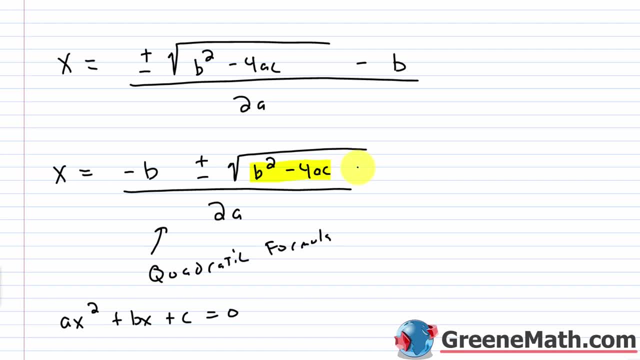 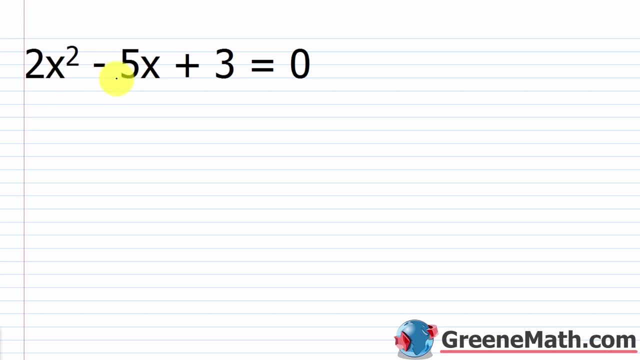 two real solutions And if it's negative, you're going to end up with two solutions that involve that imaginary unit. i All right, So let's take a look at the first example. So we have 2x squared minus 5x plus 3 equals zero. 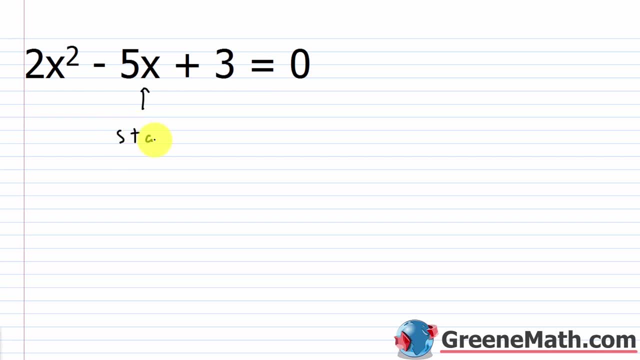 So this is already written in standard form. force. This is in standard form. So if it's not in standard form, the first thing you got to do is write it like this Again: ax squared plus bx plus c equals zero. So what you got to get used to is just kind of matching things. 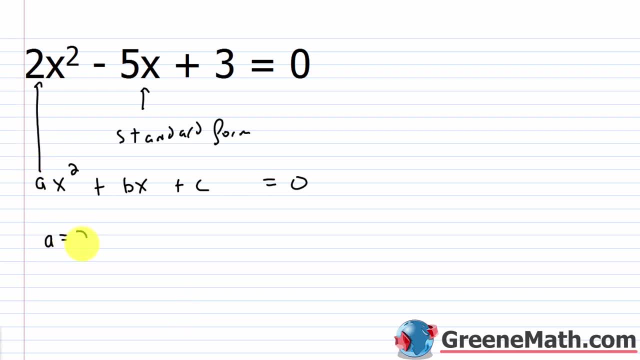 right. So a here is 2.. So a is equal to 2.. b here is negative 5.. So b here is negative 5.. And the sign is very important, Remember I could write this as plus negative 5, like that. So b is negative. 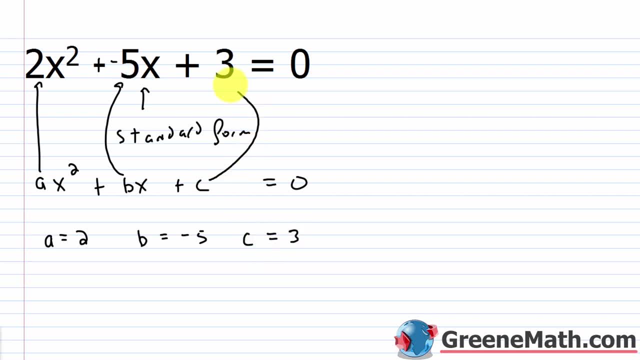 5.. And then c is equal to 3, right c is 3.. So I'm going to take these inputs and just plug it into the quadratic formula And I'm going to have my answer really, really quickly. Again for the 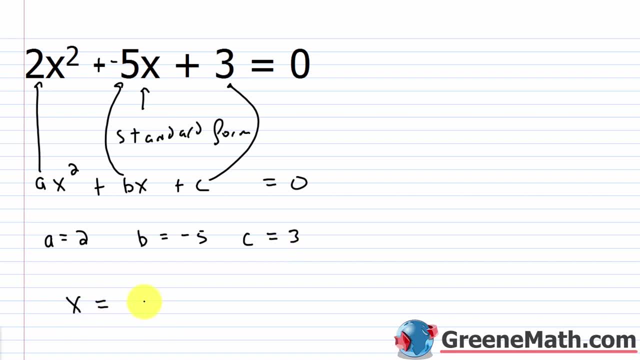 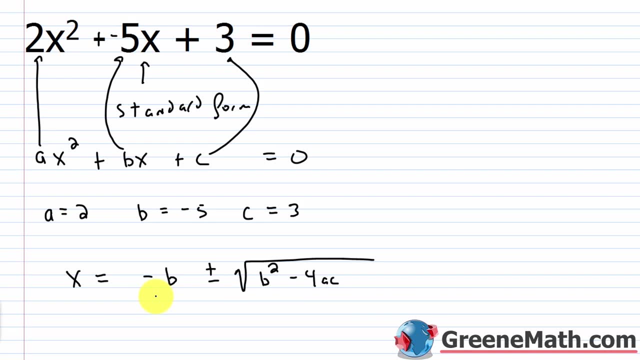 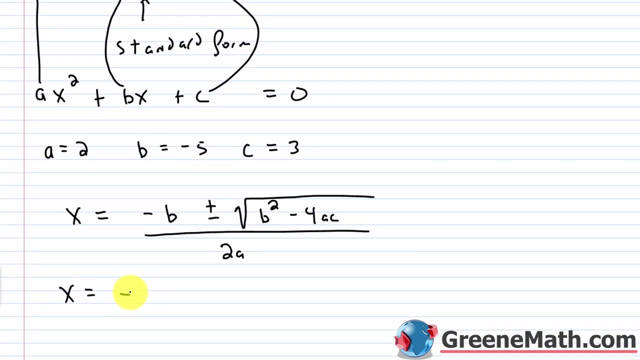 quadratic formula: x is equal to negative b Plus or minus the square root of b squared minus 4ac, all over 2a. All right, So again, I'm just going to plug in. So we'll have: x is equal to negative For b, I have negative 5.. So 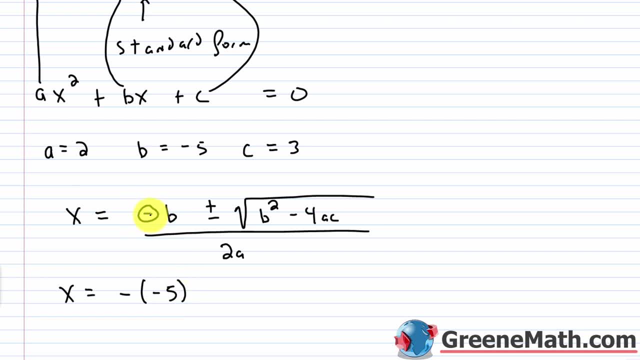 the negative of negative 5.. Again, don't confuse the signs. That's a negative out in front, This is a negative 5.. Then, plus or minus the square root of You have b squared. Negative 5 squared is 25 minus 4 times. 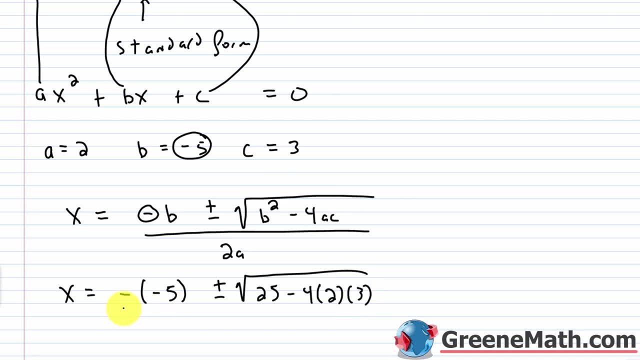 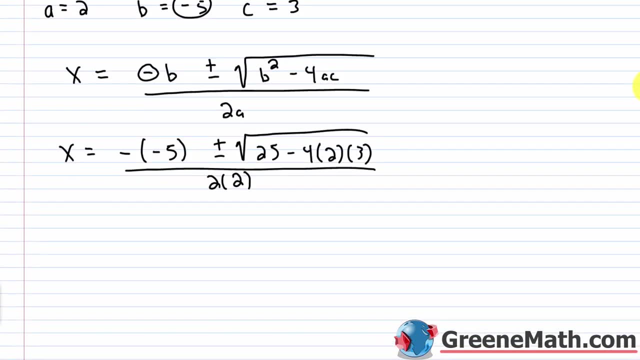 For a, you have 2.. For c, you have 3.. And then this is all over 2 times a. So 2 times For a, we have 2.. All right, Let's scroll down a little bit. So x is equal to what? x is equal to the. 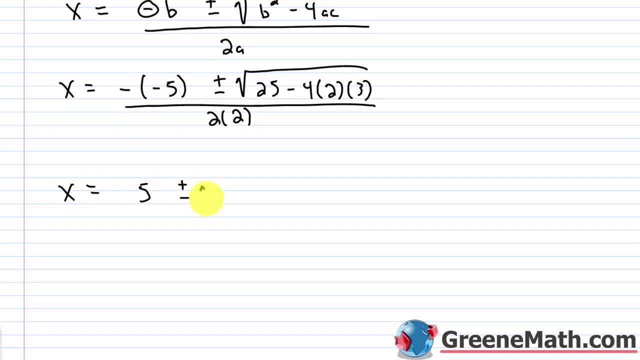 negative of negative 5 is 5.. Then plus or minus the square root of We'll have: 25 minus 4 times 2 is 8.. 8 times 3 is 24.. This is 24.. And this is all over 2 times 2, which is 4.. 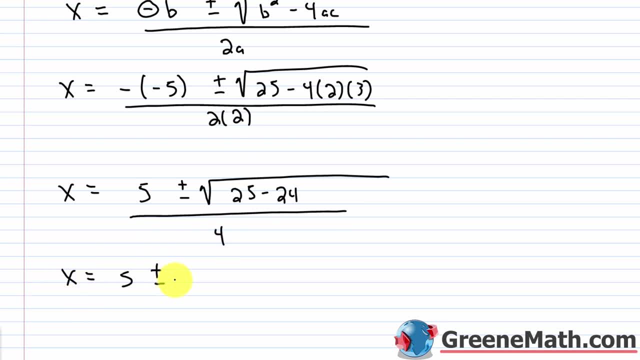 So then x is equal to. You have 5 plus or minus. the square root of 25 minus 24 is 1.. So you have the square root of 1 there over 4.. And then let's scroll down a little bit more, So then we'll have: 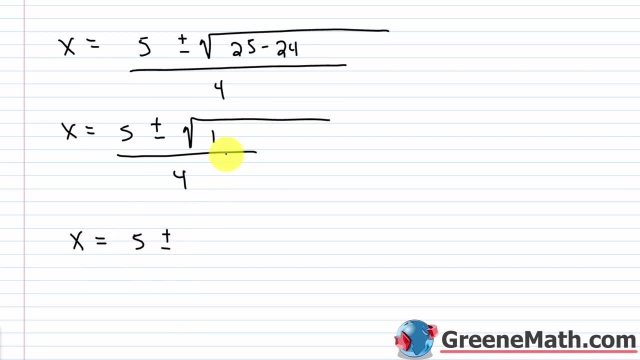 x is equal to 5 plus or minus. We know the square root of 1 is 1.. And then this whole thing is over 4.. So this is going to give us two different solutions. You have: x is equal to 5 plus 1 over. 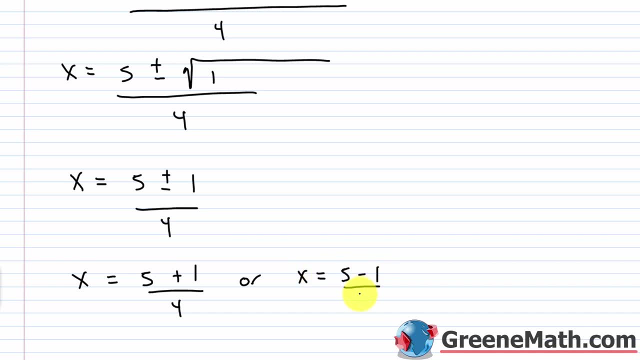 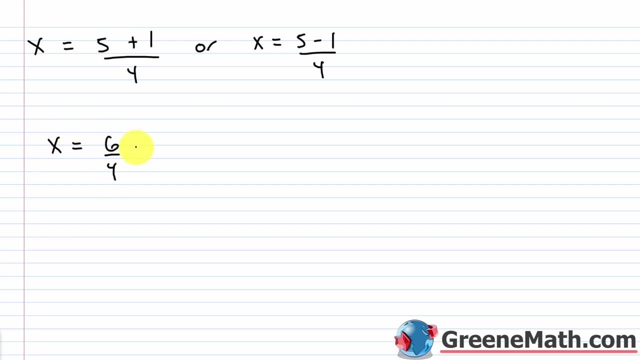 4.. And then you also have x is equal to 5 minus 1 over 4.. So your two solutions here: 5 plus 1 is 6.. 6 over 4.. You have x is equal to 6 over 4, which is going to reduce to what They're each. 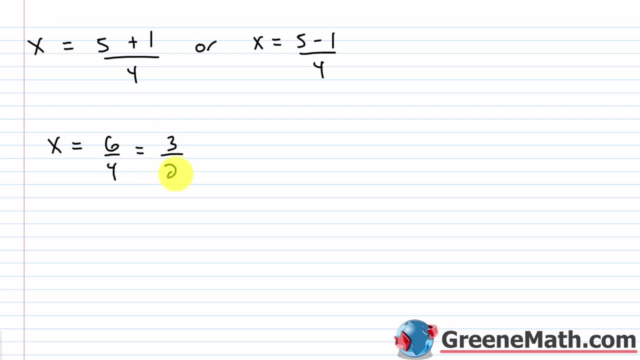 divisible by 2.. 6 divided by 2 is 3.. 4 divided by 2 is 2.. So x equals 3 halves. Or 5 minus 1 is 4.. 4 over 4 is 1.. So x is equal to 1.. So in solution set notation we'll write: 1 comma 3 halves. 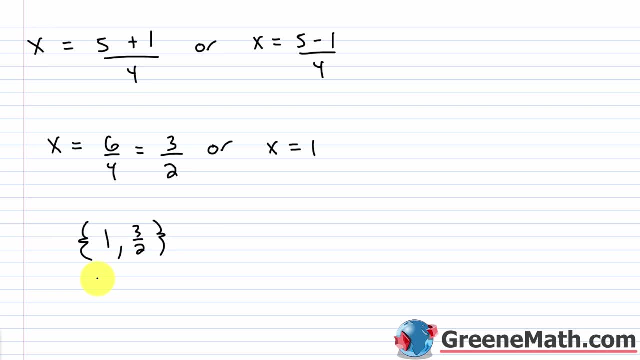 Now you can pause the video, You can go back and you can check And you can verify that 1 works as a solution and that 3 halves works as a solution. The other thing you might notice is that this 2x squared minus 5x plus 3 equals 0 is factorable, So you might want to solve it using. 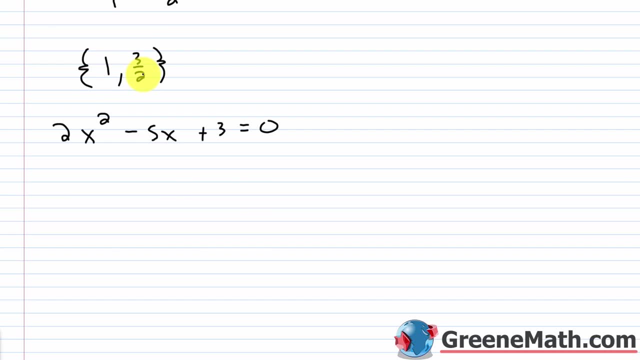 factoring and verify that you get these as the same answer. So if I was to factor this guy, what would I get? Well, this is a 2x squared, So I'd put 2x here and x here. Now, what goes here and here? Well, 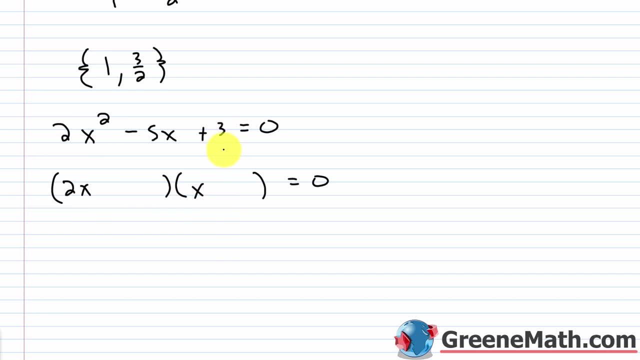 my final term is a 3.. Now don't just go with 3 and 1, because again the middle term is negative. So that means I'm going to need a negative 3 and a negative 1, because negative times negative will. 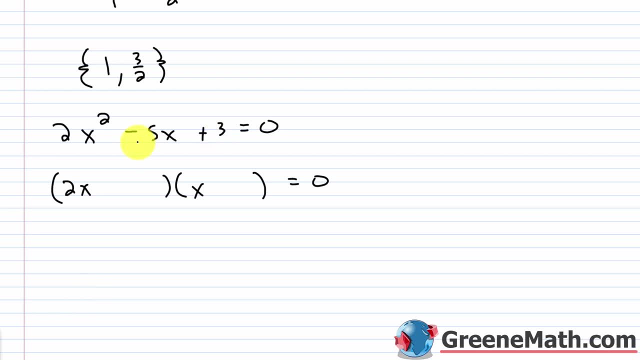 give me that positive there And negative plus negative will give me a negative there. So I've got to make sure I line this up right. I want to put a negative 3 here and a negative 1 here, So that would be the correct factorization, because the outer 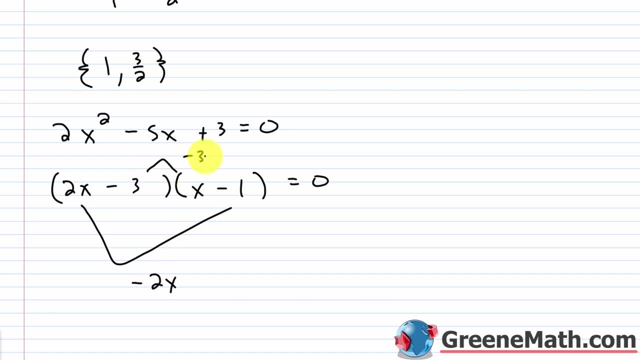 will be negative 2x and the inner would be negative 3x. Negative 2x plus negative 3x is negative 5x. You can eyeball this and see that this guy right here. if we solve it by factoring. 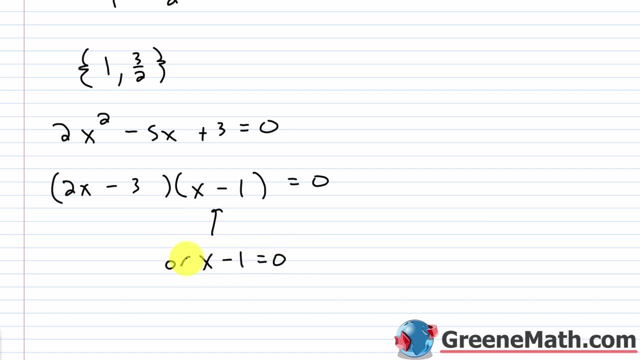 you have x minus 1 equals 0, or you have 2x minus 3 equals 0. Those are your two factors, And if we solve each of these, you add 1 to each side of the equation. here you get x equals 1.. 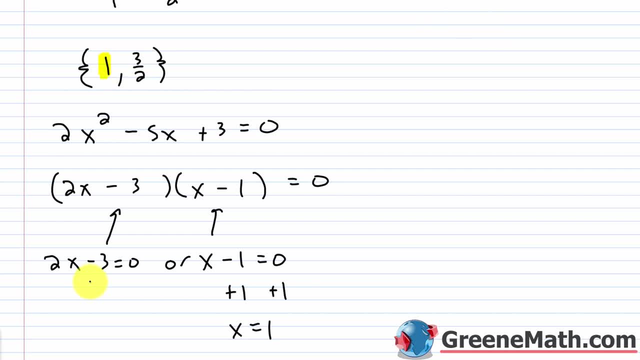 That's exactly what we got right there. If you solve this guy, you get x equals 1.. If you solve this guy, you get x equals 1.. If you solve this guy, you add 3 to both sides of the equation, You get 2x is equal to 3.. 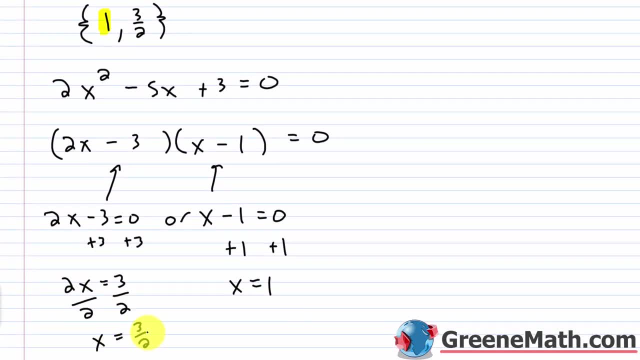 Divide both sides by 2. You get x equals 3 halves, And again, that's exactly what we got right there. So you can see that whether you use factoring or the quadratic formula, you get the same result, And you could complete the square if you wanted to. It's all going to give you the 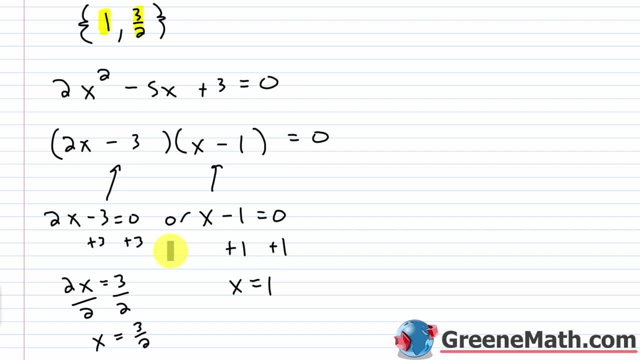 same answer. It's just a matter of what your personal preference is, And I know for most students, once they learn the quadratic formula, it's just something they're going to use forever. Right, The quickest and easiest method to use in most situations. 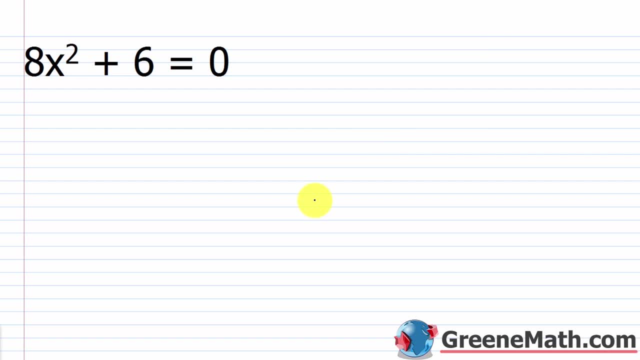 All right, let's take a look at another one. So suppose you saw 8x squared plus 6 equals 0.. So you might say, well, I'm missing my bx term, right, My term where I have x to the first power. 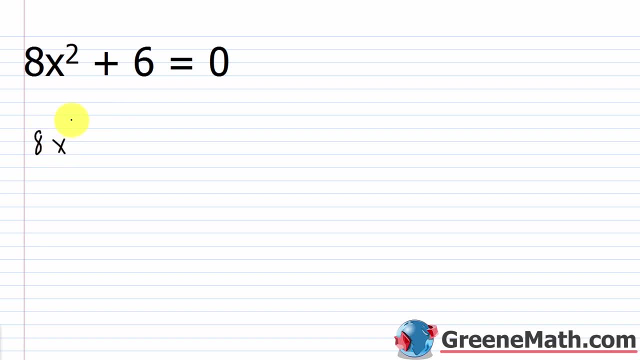 Well, that's OK. You could rewrite this and say: you have 8x squared plus 0x plus 6 is equal to 0.. Remember this guy. this guy and this guy are allowed to be any number of times 0.. 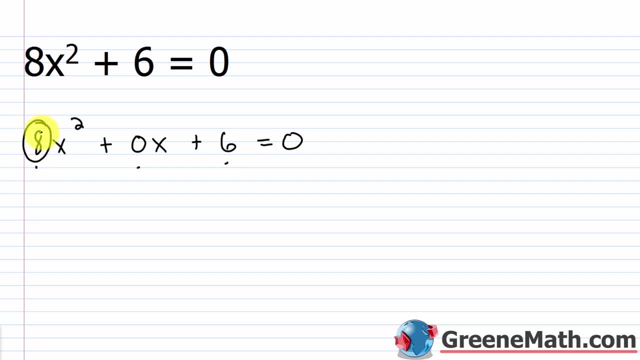 However, we can create any real number that you choose, with the one exception that this guy cannot be zero. We never said that this guy couldn't be zero, only that this guy could be. So my A is going to be equal to 8.. That's the coefficient for x squared. 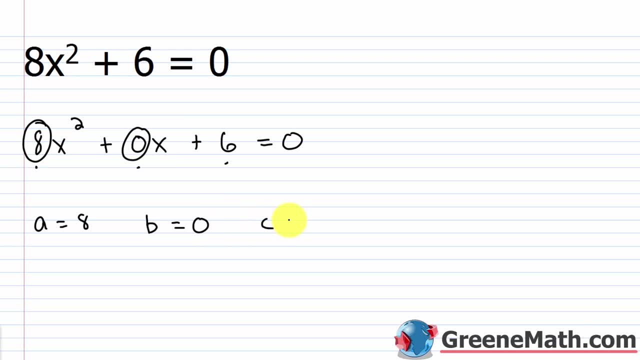 My b is going to be equal to 0.. That's my coefficient for x to the first power, And my c is going to be equal to 6.. That's my constant. Again, all I'm going to do is I'm just going to plug in. 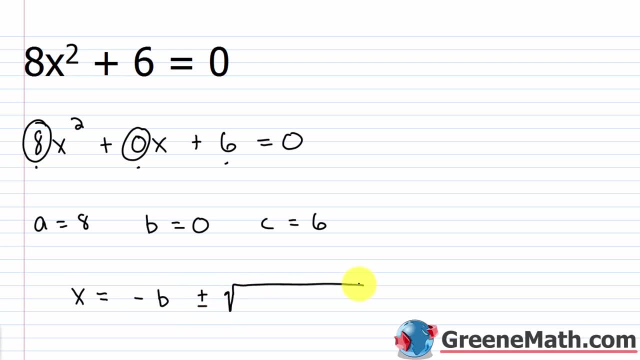 So x is equal to or minus the square root of b. squared minus 4ac, this whole thing is over 2a, So let's plug in. we want to plug in a 0 here. we want to plug in a 0 here. we want to plug in an 8: here we want to. 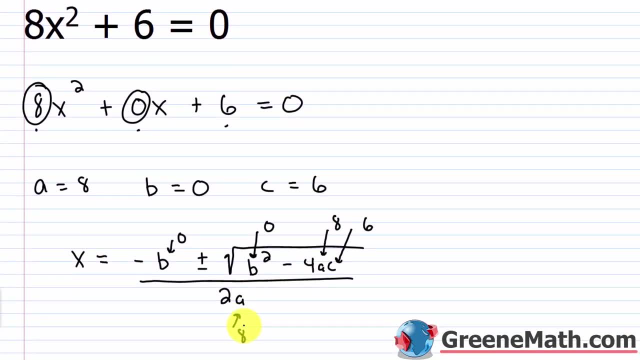 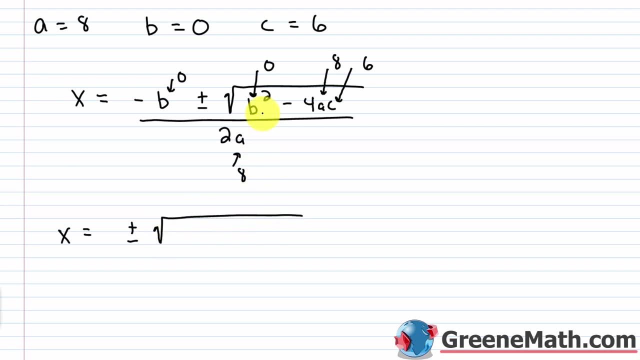 plug in a 6 here. we want to plug in an 8 here, So we'll have: x is equal to negative, 0 is just 0. then plus or minus, the square root of 0 squared is 0. so minus 4 times 8 times 6, and this is all. 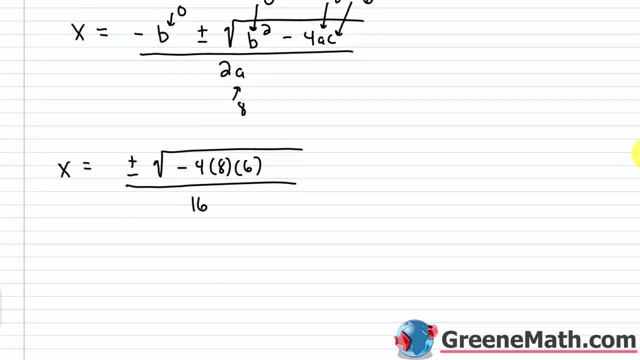 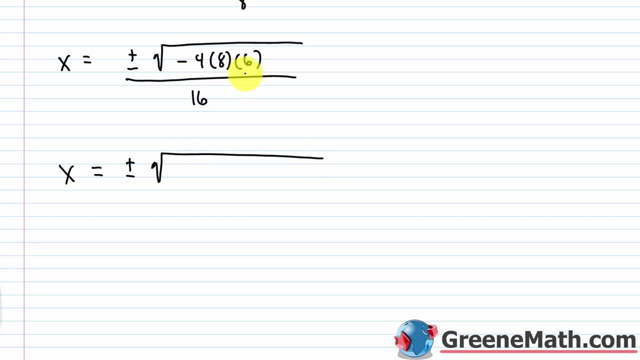 over 2 times 8, which is 60.. Let's scroll down, get a little bit more room, So we'll have: x is equal to plus or minus the square root of now. before we go through a multiply, we know this is not going to be a perfect square, so let's just separate this up into negative 1 times 4.. 4 is a perfect. 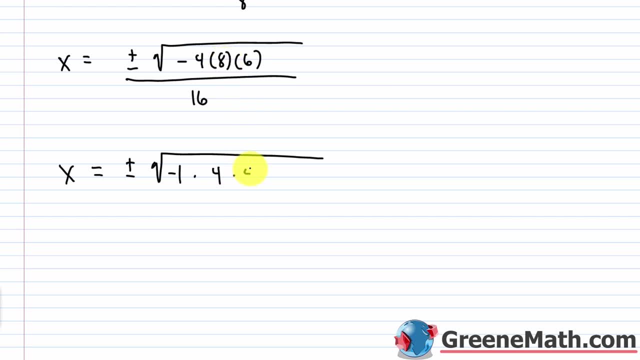 square, and then let's take 8 and break it up into a square root of 0. So we'll have: x is equal to negative 0, and we're going to divide this up into 4 times 2.. 4 times 2, 6 is 3 times 2, so it's. 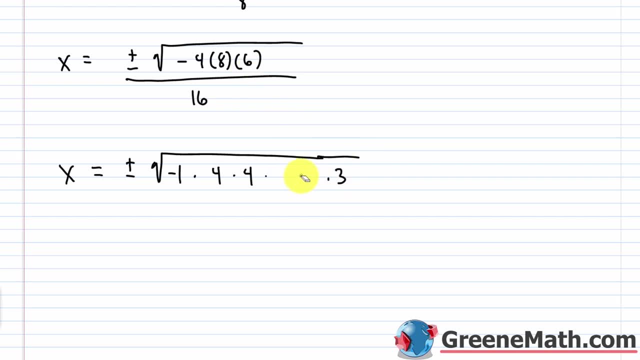 times 2 times 3.. This I can go ahead and combine and say: this is 4 and so what am I going to be left with? this is over 16.. We'll have a 4, a 4 and a 4.. I know that each 4 can be pulled out Square. 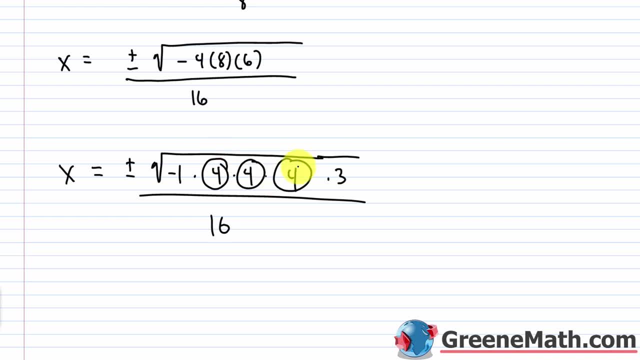 root of 4 is 2.. So this is essentially 2 times 2 times 2, which is 8.. So x is going to be equal to plus or minus 8 times the square root of 0, squared times 4 times 2.. So this is going to be: 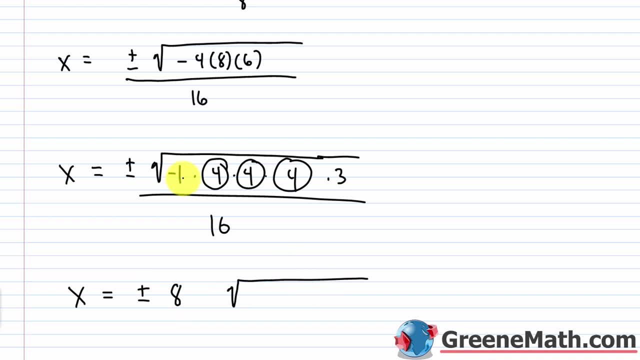 of now negative 1 that can come out. square root of negative 1 is i, so plus or minus 8. i times the square root of what's going to be left is a 3 and then this is over 16. now i can cancel between: 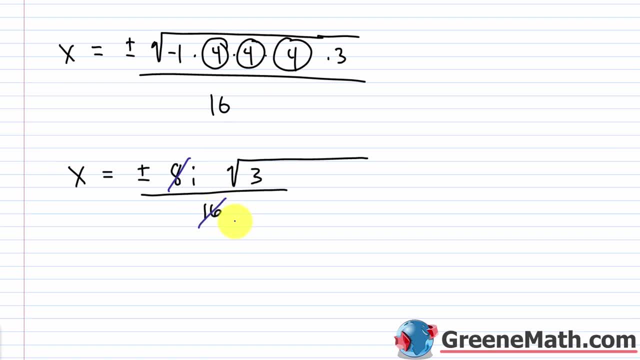 numerator and denominator. here i have this 8 that can cancel with this 16, so this would be a 2. so in the end i'd end up with: x is equal to plus or minus. i times the square root of 3 all over 2. 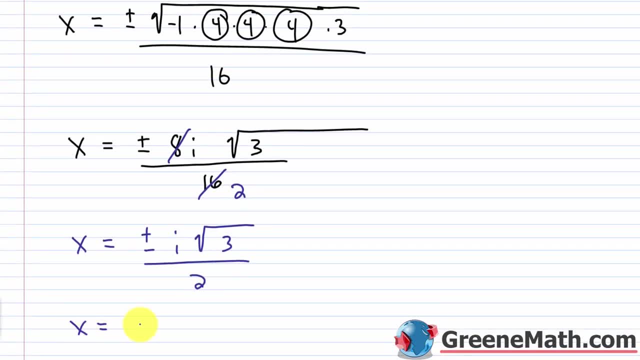 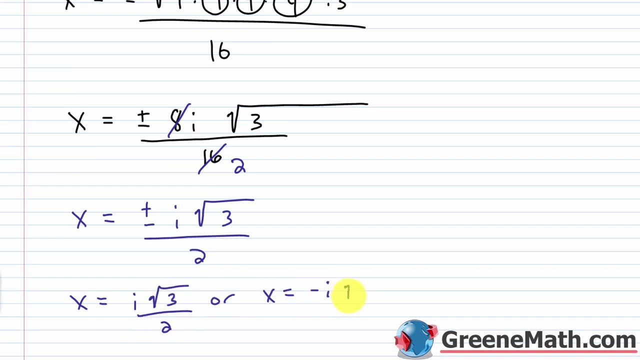 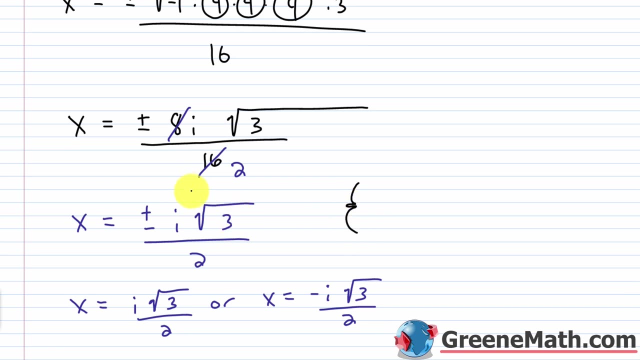 so two separate solutions, right you have. x is equal to: i times square root of 3 over 2, or x is equal to negative, i times square root of 3 over 2. but again, this is kind of the shorthand way to write that. and then for solution set notation, why don't we go ahead and use this: 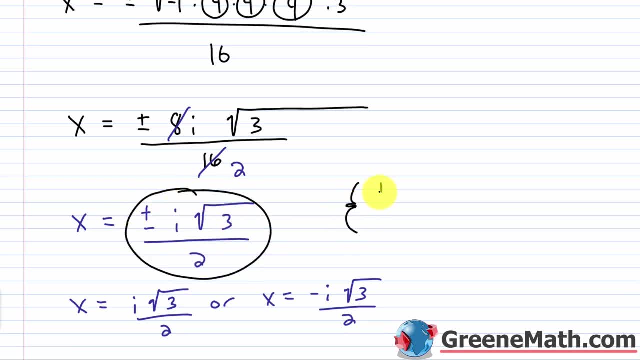 compact one right here. so inside my separators, let's say we have plus or minus. i times the square root of 3 over 2 and again, feel free to check this, you can just point the item and find the answer to that question. so in this case, so x is equal to 1. 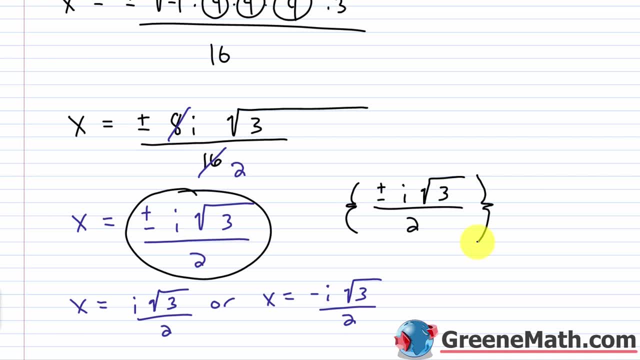 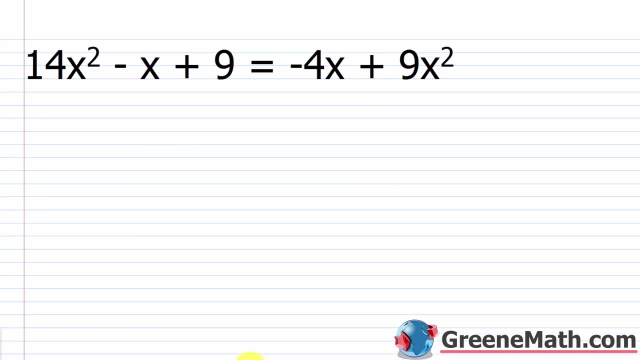 pause the video, plug it in and verify that you get the correct answer. you have two different solutions to check, but it's going to be something that's going to be a little bit tedious for you to do. Well, let's take a look at another example. 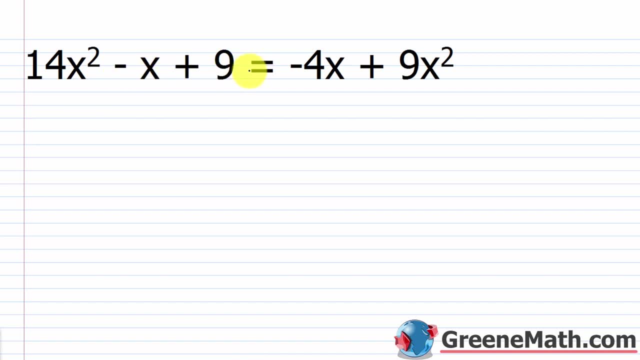 So we have 14x squared minus x plus 9, and this is equal to negative 4x plus 9x squared. So the biggest mistake that students make is they would see something like this and say, okay, I'm going to plug in a- 14 for a, I'm going to plug in a negative- 1 for b- and 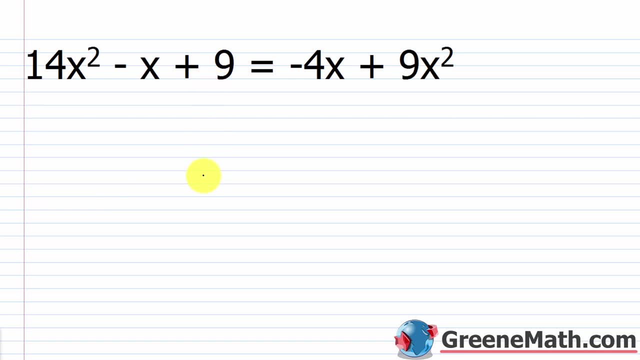 a 9 for c. Now you have to put this in standard form. So you want the left side to look like this: Something times x squared, plus something times x plus some constant, and this is equal to 0. So the right side is 0, the left side looks like this: 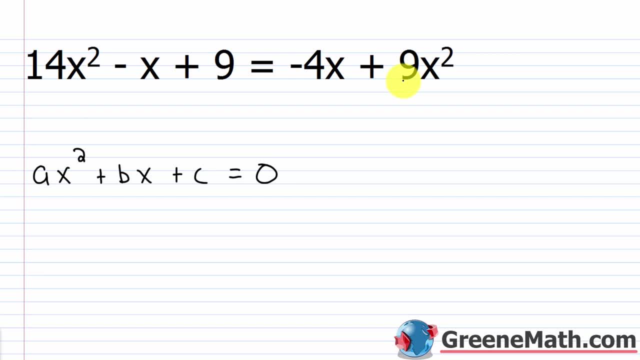 That's not what we have here, So we need to kind of manipulate this a little bit. We would add 4x to each side of the equation and we would subtract away 9x squared from both sides of the equation. So what that's going to give us, this would cancel and become 0.. 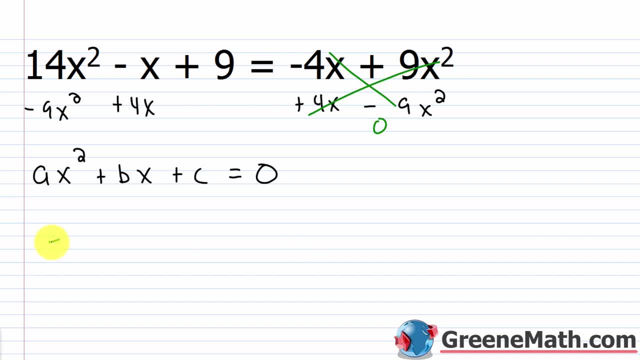 On the left side, 14x squared minus 9x squared would be 5x, squared, Then negative x plus 4x would be positive 3x, then plus 9, and this equals 0.. So this is now in standard form and something we could just plug into the quadratic formula. 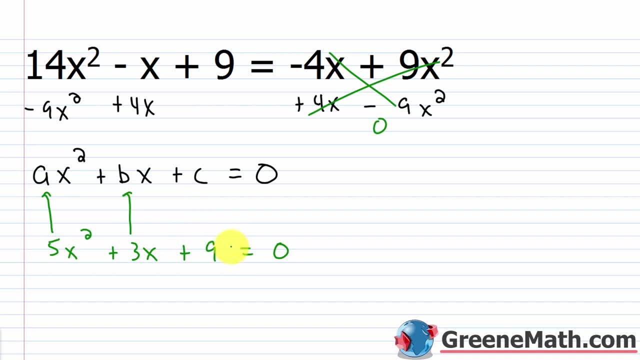 So we could take 5 and plug it in for a, 3 and plug it in for b, and 9 and plug it in for c. So a equals 5,, b equals 3, and c equals 9.. So what's the quadratic formula? 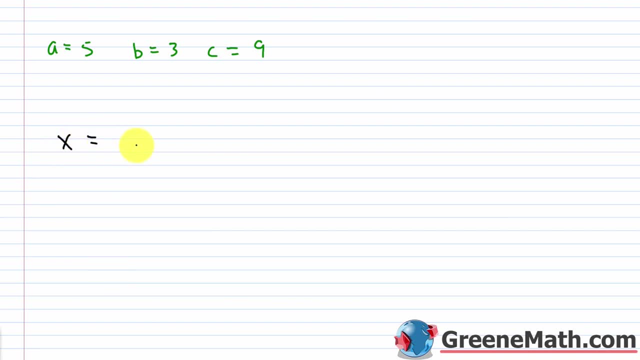 At this point you should start to memorize it. It's x is equal to. you have negative b plus or minus the square root of b squared minus 4ac. all of this is over 2a. So again I'm plugging in a, 5 for each a. 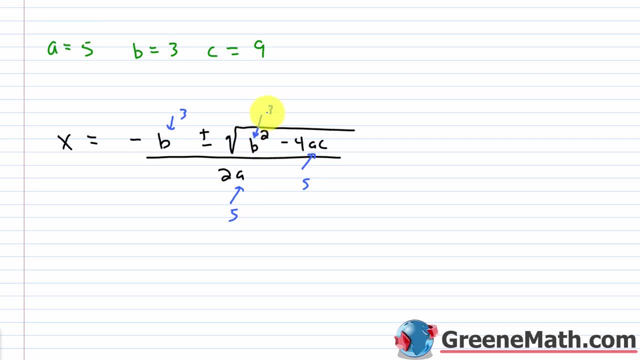 I'm plugging in a- 3 for each b, I'm plugging in a- 3 for each b And I'm plugging in a- 9 for the c. So what we'll have? we have: x is equal to negative 3 plus or minus. the square root of 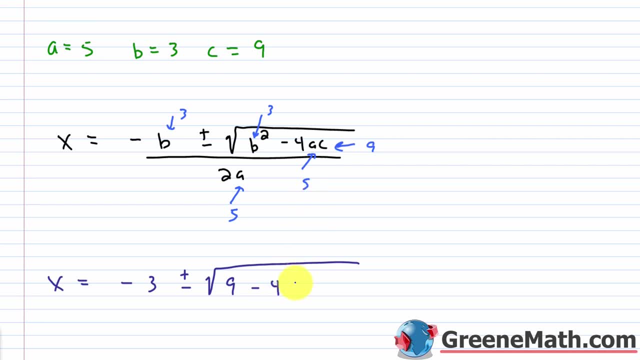 3 squared is 9 minus 4 times, you have 5 times 9.. Okay, this is all over 2 times 5, which is 10.. Alright, so we're going to have: x is equal to. You have negative 3.. 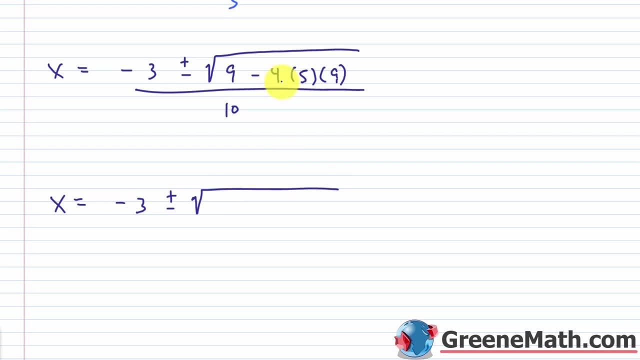 You have negative 3 plus or minus. the square root of 4 times 5 is 20,. 20 times 9 is 180.. So if you had 9 minus 180, that's going to give you negative 171,. then again, this is: 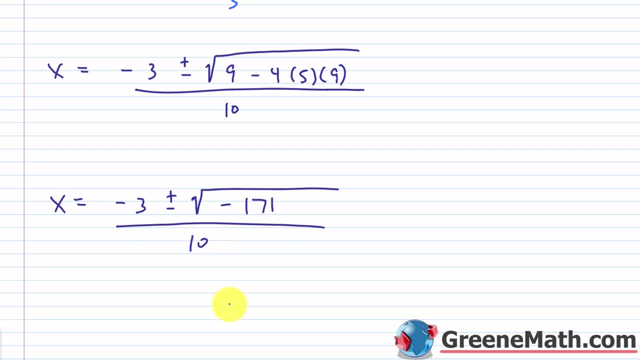 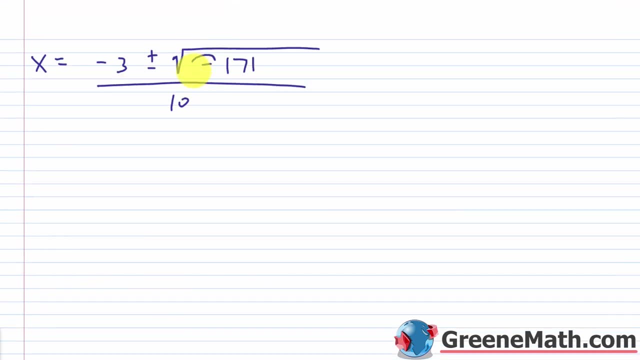 all over 10.. So how do we simplify this? Because we're not done. we can make this look a little better. Let me copy this. we'll bring it to the next page. So realize that if you see a negative inside of the square root symbol, you can pull out. 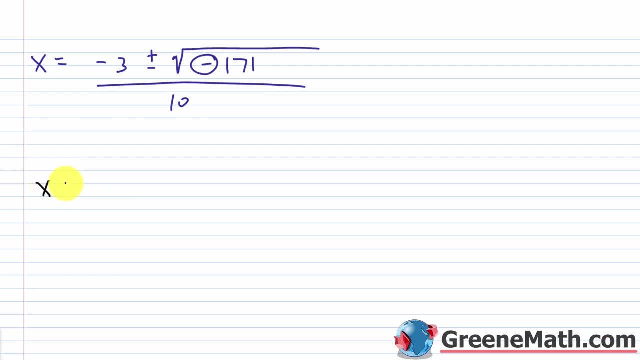 an i. So let's start by just doing that. Let's say this is: x is equal to negative 3 plus or minus. i times the square root of 171.. Now, before I write that, what is 171?? What would that factor into? 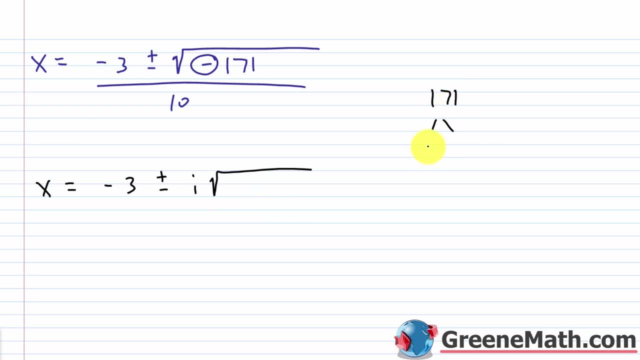 Well, 1 plus 7 is 8,, 8 plus 1 is 9.. So I know it's divisible by 9.. It would be 19 times 9.. 9 times 10 is 90, plus 9 times 9, which is 81,. 81 plus 90 would be 171. 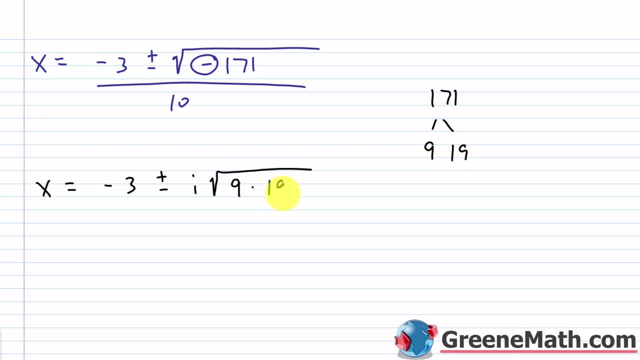 So I could write the square root of 9 times 19 like that: Okay, This is all over 10.. We know this guy is a perfect square, so the square root of 9 is 3, I could pull that out. 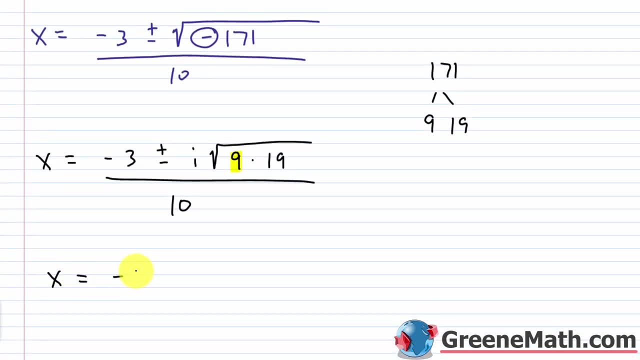 So we could say that we have: x is equal to negative 3 plus or minus 3i times the square root of 19, and this is all over 10.. Now again you could leave it like this, but again you want to realize this is two different. 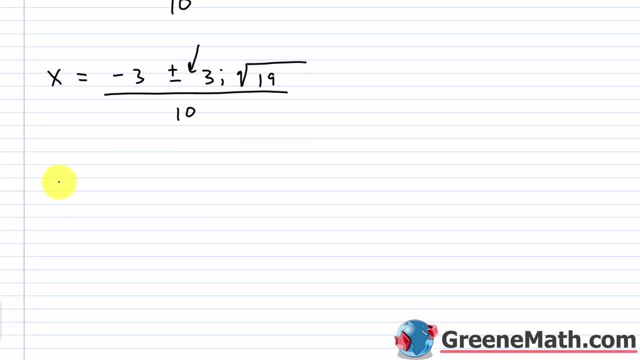 solutions. This turns out to be what It turns out to be. x is equal to negative 3i, Negative 3i plus 3i times the square root of 19 over 10.. And then also you have x is equal to negative 3 minus 3i times the square root of 19 over. 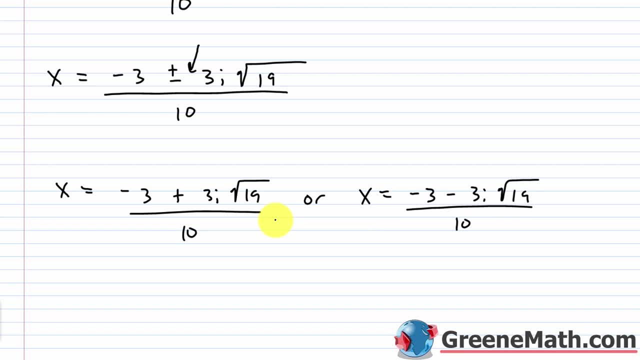 10.. Okay, Those two different solutions In solution set notation. we'll just write this in the more compact form. so: negative 3 plus or minus 3i times the square root of 19, all over 10.. And then we're done. 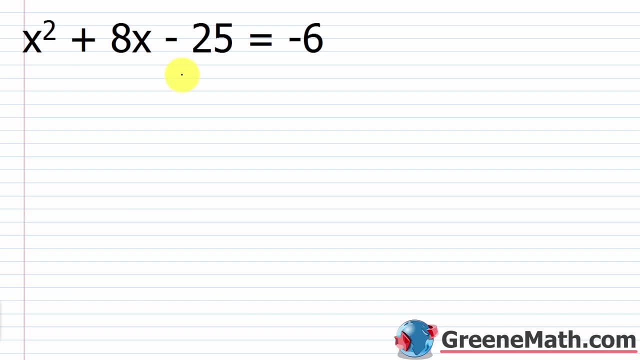 All right, Let's take a look at another. So we see x squared plus 8x minus 25 equals negative 6.. Again, we want this in standard form, so we would just add 6 to each side of the equation. 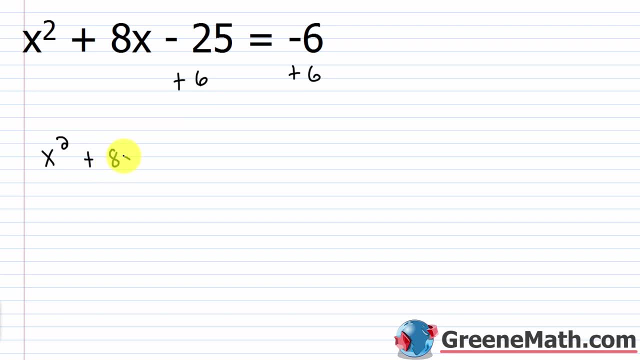 So that would give us x squared plus 8x, then negative 25 plus 6 would be negative 19,. so minus 19.. And this equals 0.. So now this matches: our ax squared plus bx plus c is equal to 0, where a is going to. 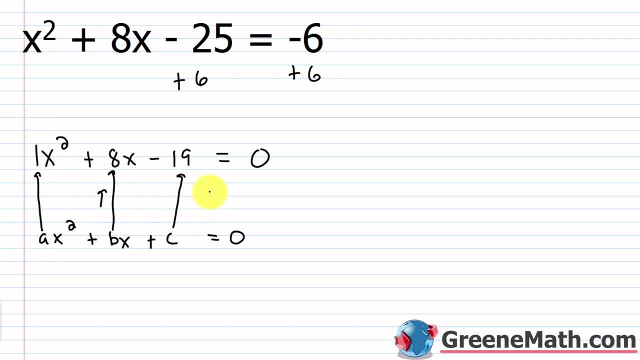 be 1.. b is going to be 8.. And c is going to be negative 19.. So a is 1,, b is 8, and c is negative 19.. And again, once you get good at this, you just kind of eyeball things and plug in and 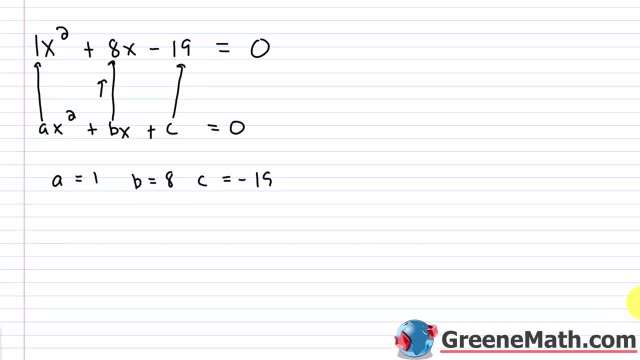 you're basically done with the problem in a few minutes. So we'll have: x is equal to negative b, B is 8, so negative 8 plus or minus the square root of b squared B is 8.. So if I squared 8, I'd get 64.. 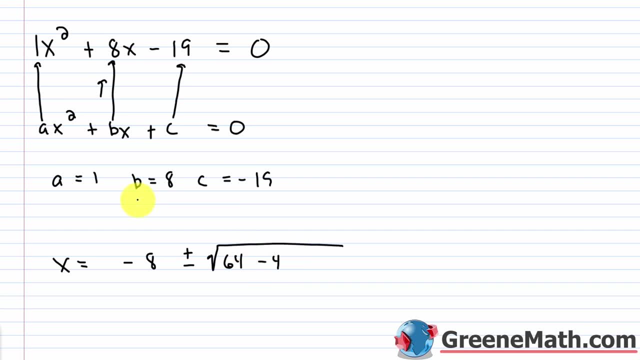 Okay, So that's going to be minus 4 times a: a is 1, times c: c is negative 19, and this is all over 2 times a. Again, a is 1,, so this is just 2.. 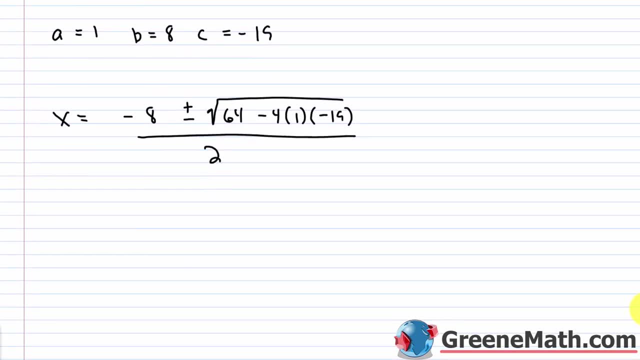 All right. So what do we have here? We'll have: x is equal to negative 8 plus or minus the square root of you have 64, then negative 4 times 1 times negative 19 is going to be 76.. 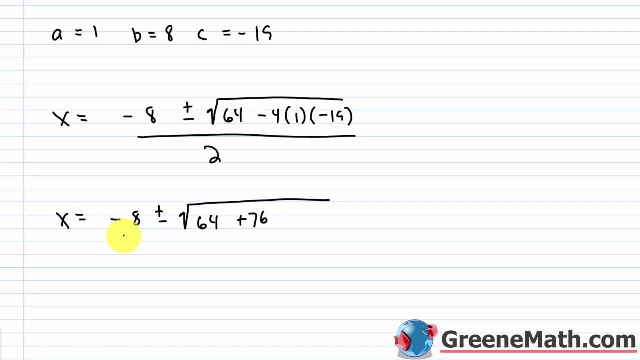 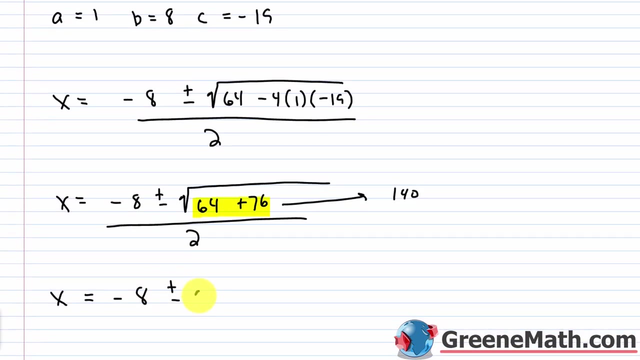 If you had 64 and 76, what are you going to get? It's going to give you 140.. So the result of this right here is going to end up being 140. So this is over 2.. So we'll have: x is equal to negative 8 plus or minus the square root of 140, all over 2.. 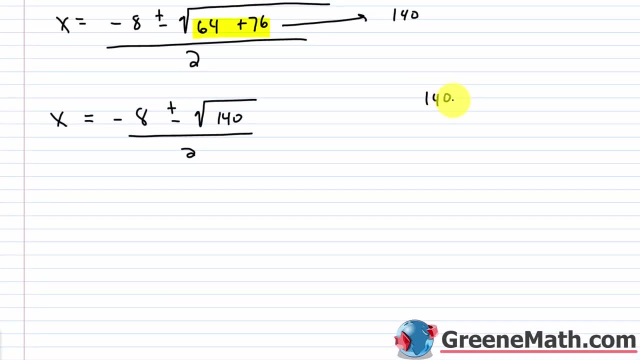 Now we're not done. We can keep simplifying. 140 is what? Well, it ends with 40.. So we know it's divisible by 4.. It would be 4 times 35. So we know it's divisible by 4.. 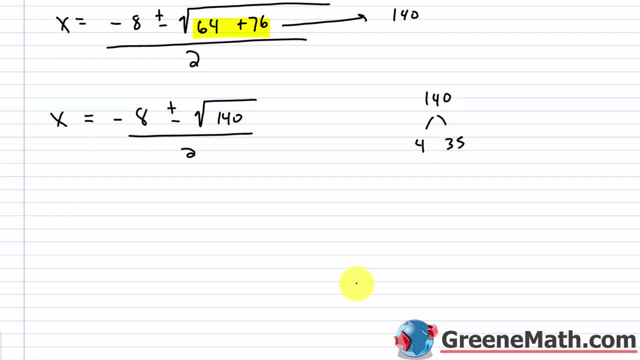 So we know it's divisible by 4.. So we know it's divisible by 4.. And 35 is 5 times 7.. So we can take this and say: this is x is equal to negative, 8 plus or minus. if I did the 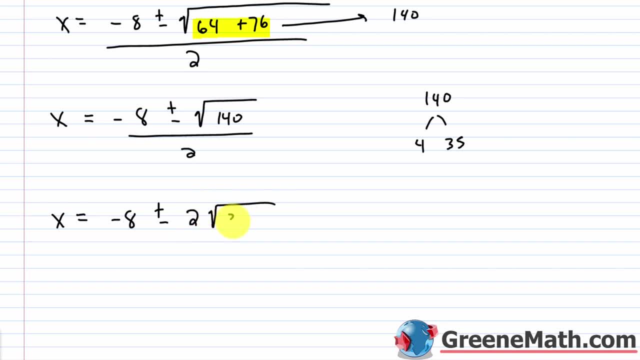 square root of 4, that would be 2, then times the square root of 35. Can't really make that any simpler. Then this is over 2.. Now one thing we can do: we can factor out a 2 from here and here and cancel it with. 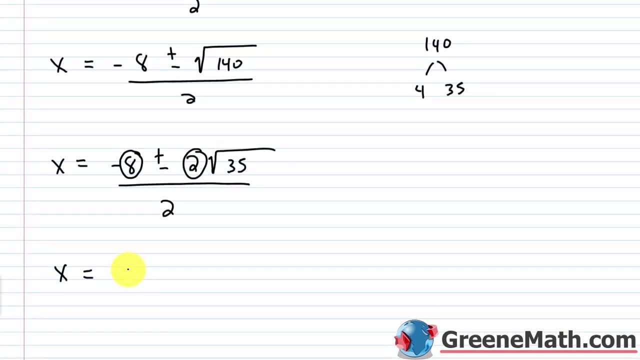 this 2.. So we could say we have x is equal to. you could say you have 2 times the quantity of 4 plus or minus the square root of 35 over 2.. And I'll cancel this 2 with this 2.. 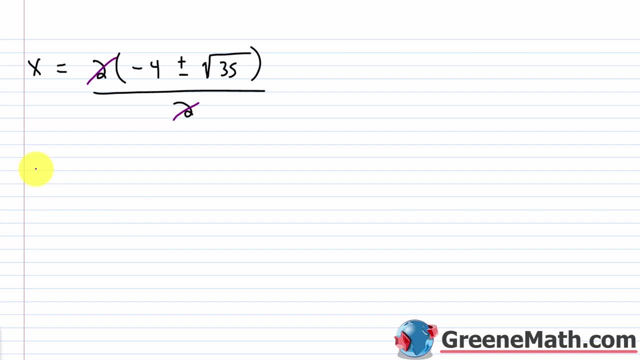 And I'll have my final answer, which will be simplified We'll have: x is equal to negative 4 plus or minus the square root of 35.. Now, whatever you want to do here, you can leave it like this, or again you could say: 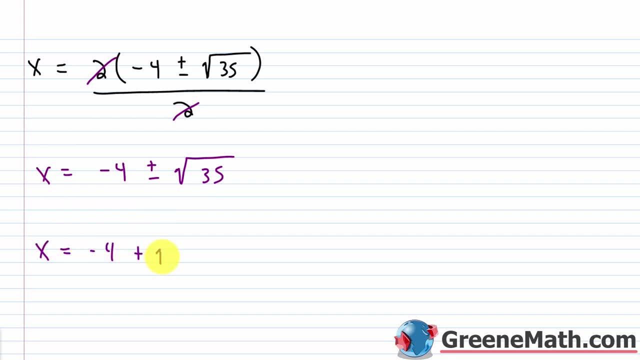 you have, x is equal to negative 4 plus the square root of 35.. Or x is equal to negative 4 minus the square root of 35.. This one and these two, it's telling you the same thing, it's just this one is more compact. 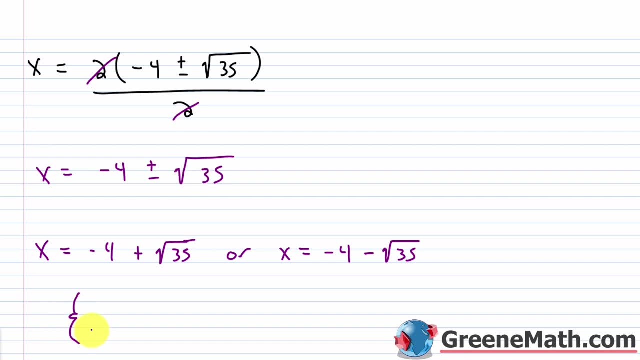 Now in solution set notation I'm just going to write that we have negative 4 plus or minus the square root of 35.. That'll be the only thing I'll put in there. Again, this notates two different solutions. Alright, for the next one. we have negative 9x squared minus 4x plus 8 equals 4.. 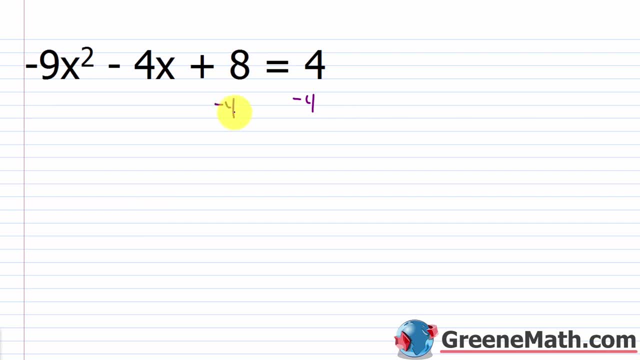 Again, very easy at this point. we just subtract 4 away from each side of the equation. We put this in standard form: It's negative. 9x squared minus 4x plus 4 equals 0.. And again, just by eyeballing this now, I should know that this is a, this is b and this is. 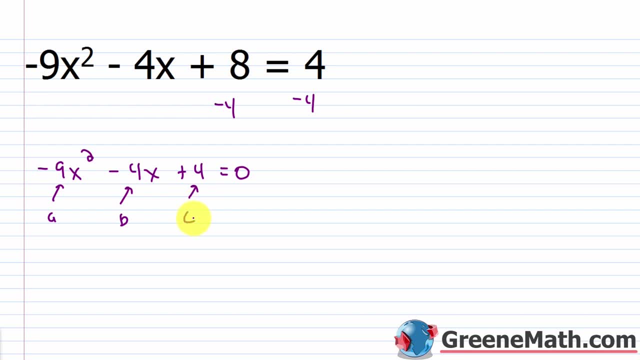 c. Alright, so a is negative 9,, b is negative 4, c is positive 4.. So I'm going to plug into my formula I have: x is equal to negative b, The negative of negative 4 is positive 4.. 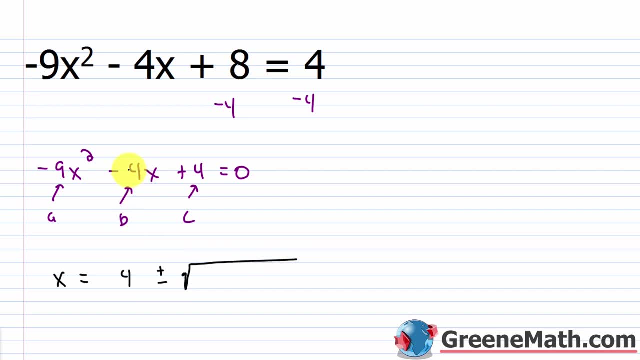 Then, plus or minus the square root of b squared negative, 4 squared is 16.. Then, minus 4 times a, a is negative 9, times c, c is positive 4.. Now this is all over. 2a a again is negative 9,. 2 times negative 9 is negative 18.. 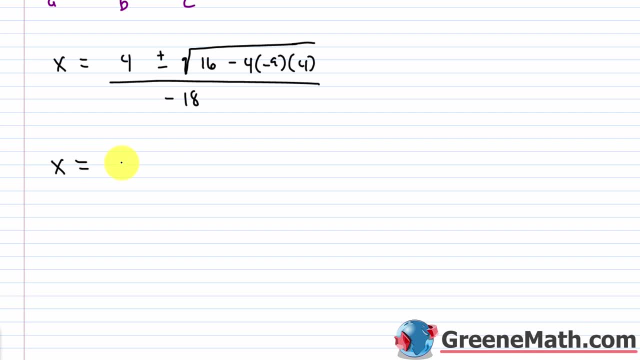 Alright, so the next thing we want to do? we have x is equal to 4 plus or minus. the square root of Negative 4 times negative, 9 is positive 36.. Positive 36 times 4 is 144.. So you would have 16 plus the result of this, which again is 144.. 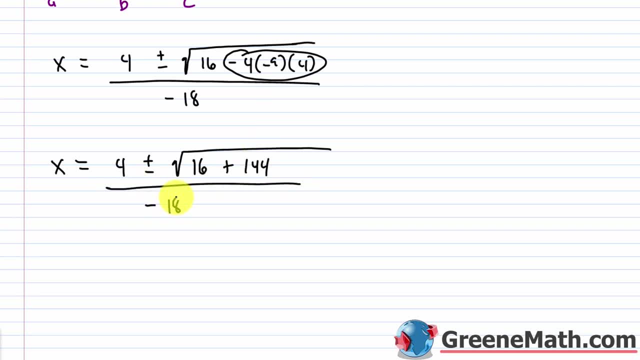 And this is all over negative 18.. So 144 plus 16 is 160.. So this would be: x is equal to 4 plus or minus the square root of. Let's write 160 as 16 times 10.. We know, 16 is a perfect square. 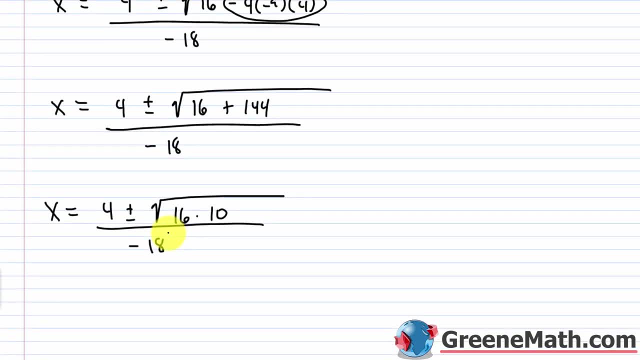 And again, this is all over negative 18.. Square root of Square root of 16 is 4, so let's write: x is equal to 4 plus or minus 4 times the square root of 10.. This is all over negative 18.. 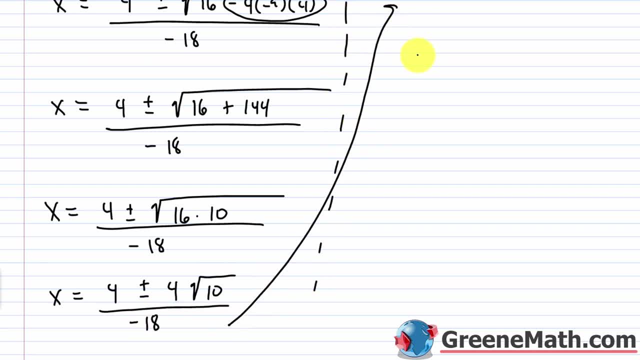 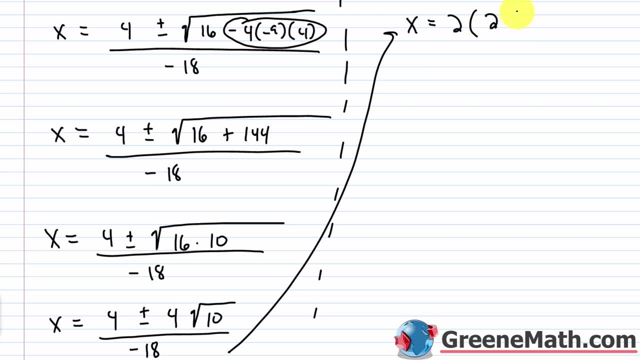 Now we can simplify this. let me drag this up. here We go. x is equal to- I could factor out a: 2. So 2 times the quantity 2 plus or minus 2 times the square root of 10 over negative 18.. 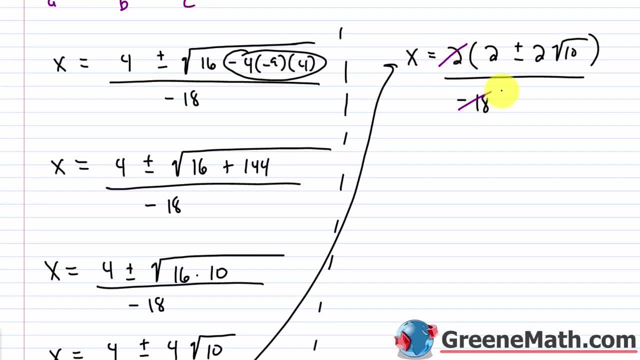 I could cancel a common factor of 2 between here and here, So this would be negative 9 now, And what we'll end up with is x is equal to 2 plus or minus 2 times the square root of 10 over negative 9.. 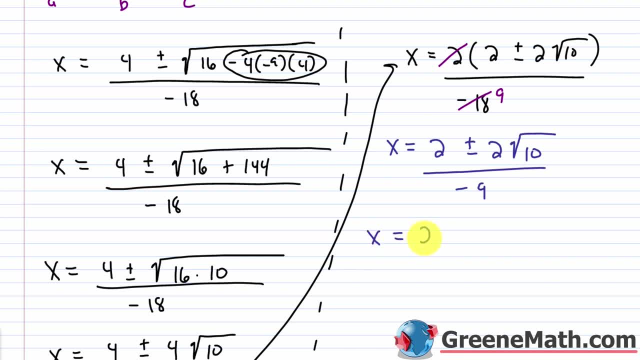 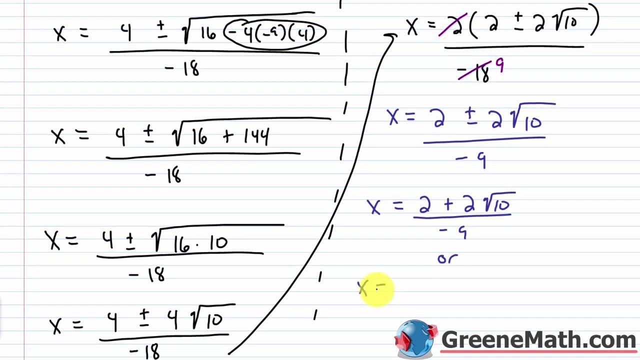 So again, this is two different solutions You'll have. x is equal to 2 plus 2 times the square root of 10 over negative 9.. Or x is equal to 2 minus 2 times the square root of 10 over negative 9.. 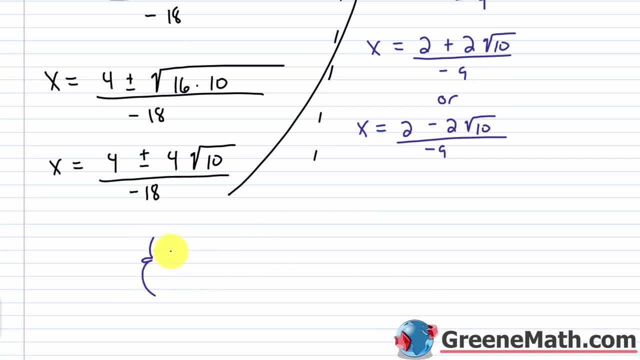 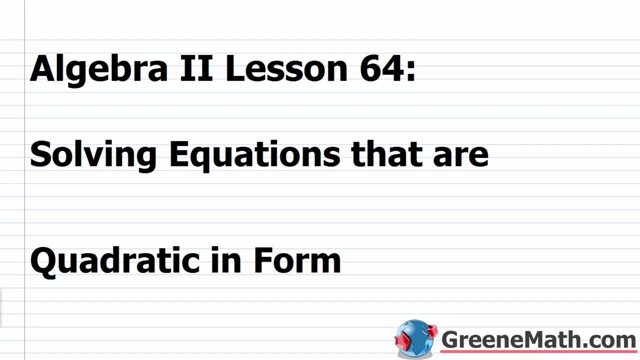 And again For solution set notation, We'll use the compact form. We'll put 2 plus or minus 2 times the square root of 10 all over negative 9.. Hello and welcome to Algebra 2, Lesson 64.. In this video we're going to learn about solving equations that are quadratic in form. 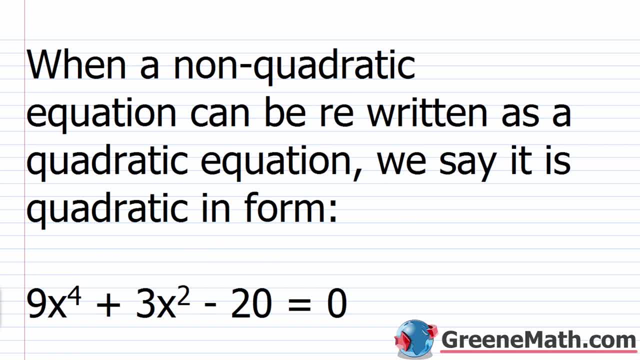 So typically you're going to see this topic come up right after you learn how to solve quadratic equations using the quadratic formula. It's a very easy topic. You might struggle with it at first Because you do have to make a little substitution, But once you kind of get that down, it's very, very easy. 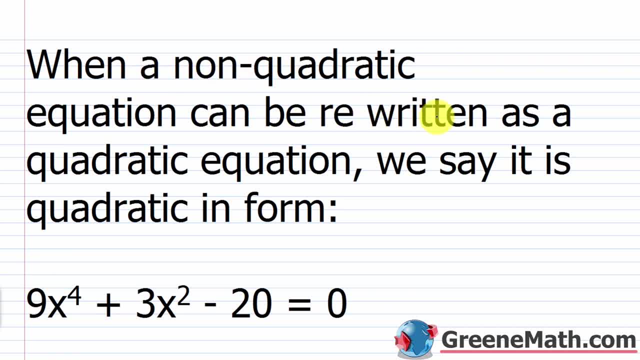 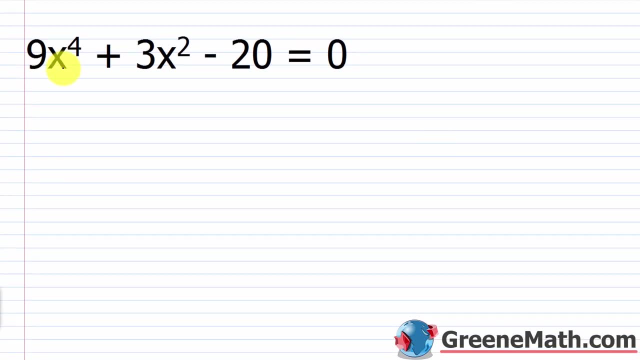 So when a non-quadratic equation can be rewritten as a quadratic equation, We say it is quadratic in form. So quadratic in form, That's what we're looking at. So as an example of this, Let's say you saw something like 9x to the fourth power plus 3x squared minus 20 equals. 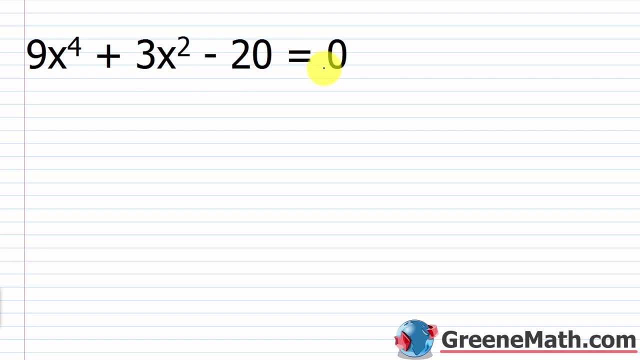 0. Well, this equation, although it's not a quadratic equation, It's quadratic in form, Meaning we could make a substitution and we could create a quadratic equation And therefore we could solve it the same way we solve a quadratic equation. Now, when you look at a generic quadratic equation, 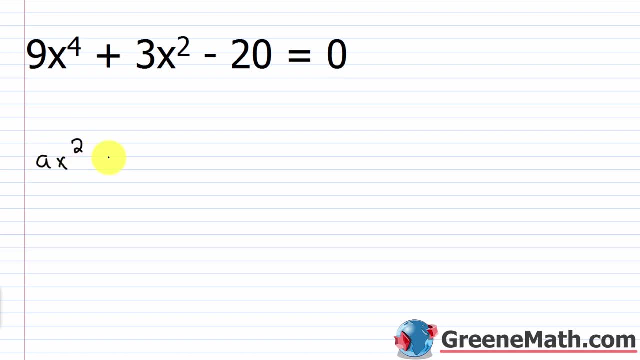 Let's say we look at ax, squared plus bx plus c equals 0. What do we see? Typically, You're going to have three terms. Now, that's not always the case, But just typically you'd see three terms. One of them is going to be a constant. 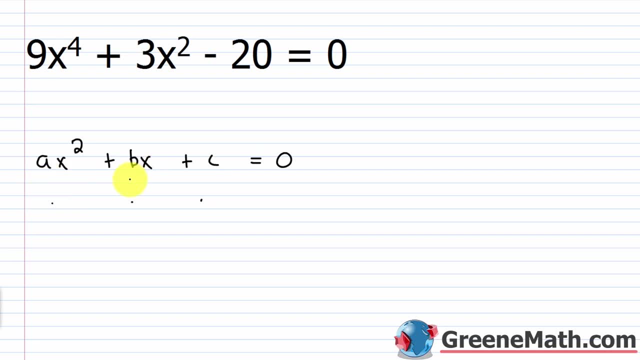 And then you're going to have generally two variable terms involved. Again, not always, But generally speaking. Now, what you want to notice here is that the variable x, that's raised to the smaller power, It's raised to the power of 1.. 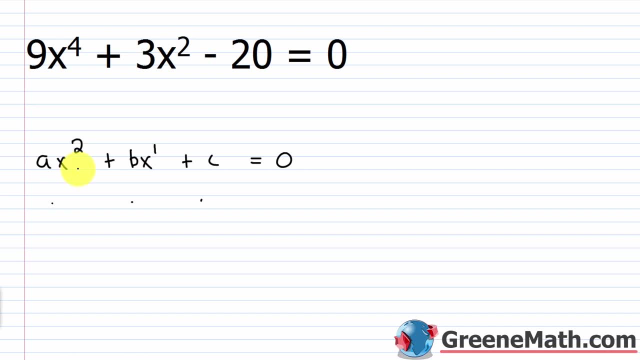 The variable x that's raised to the higher power is raised to the power of 2 or it's squared. So the higher power 2 is double that of the lower power 1.. So up here you can see the same pattern. You have three terms. 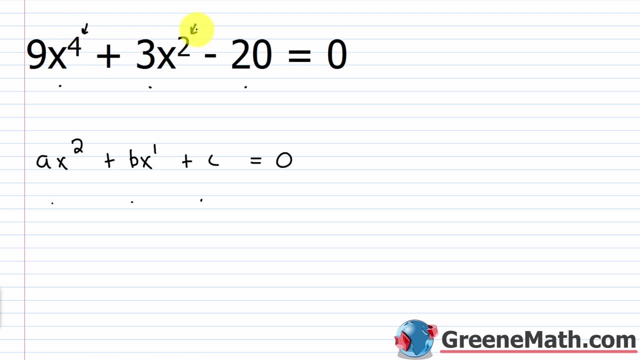 You have the higher power 4, that is double that of the lower power 2.. So what we can do when we see this again, if it's quadratic in form, We can make a little substitution and we can create a quadratic equation. So let me just erase this real quick and I want to walk you through the first one completely. 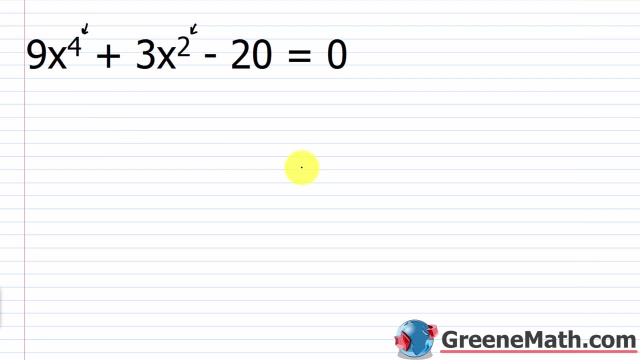 So what you want to do is you want to pick a variable. It doesn't matter what it is, just don't choose the same one in the problem. So I don't want to choose x, because that's in my problem, Let's just choose z. 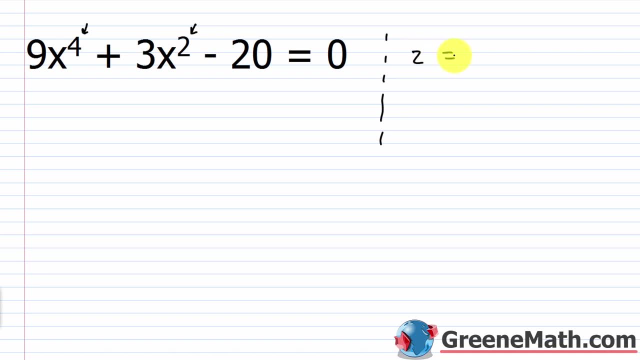 Something easy. So z is going to be equal to and it's going to be equal to the variable raised to the smaller power. So in this case that's x squared, So z equals x squared. So what I want to do is I want to go and I want to plug in a z everywhere I see x squared. 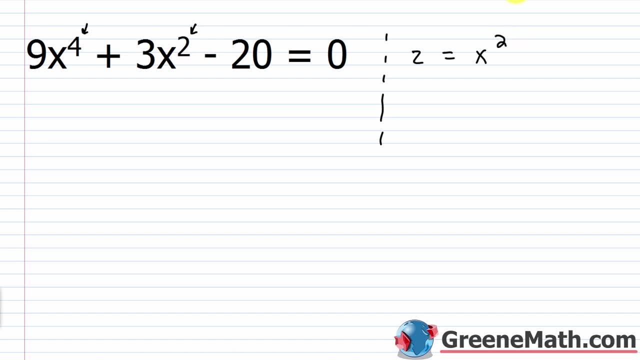 But the problem with that is- And what you kind of need to be walked through here- is that, Yeah, I only see x squared here, But by using my rules for exponents, I could create x squared squared there. This is x squared squared. 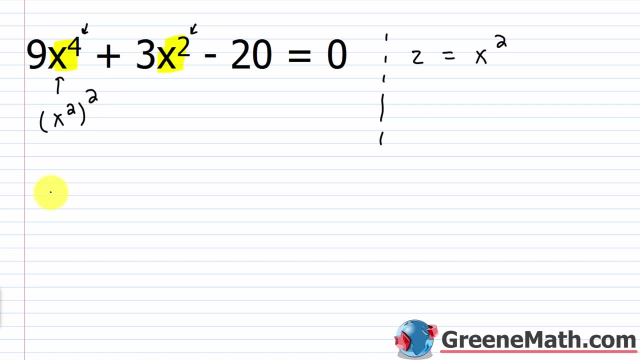 So really, I would want to rewrite this problem first and say that I have 9 x squared. squared Again by rules of exponents, x would stay the same. 2 times 2 would give me 4.. So that's x to the fourth power. 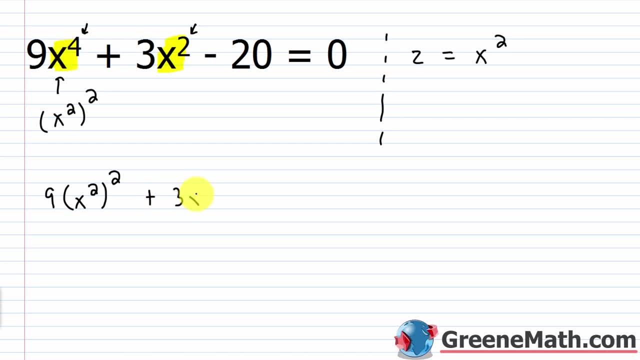 I just rewrote it. Then plus 3, x squared, then minus 20, and this equals 0.. Now, if I substitute z in everywhere I see x squared, What am I going to get? So this would be z and this would be z. 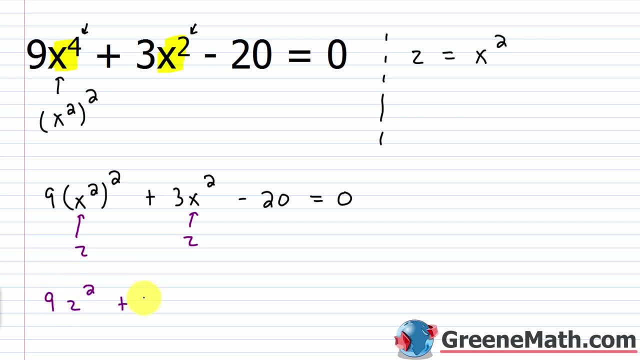 So I would have 9 z squared plus 3 z minus 20 equals 0.. So let's forget about everything above what I just wrote. Let me scroll down And let's just think about, Let's just think about the new equation that we have. 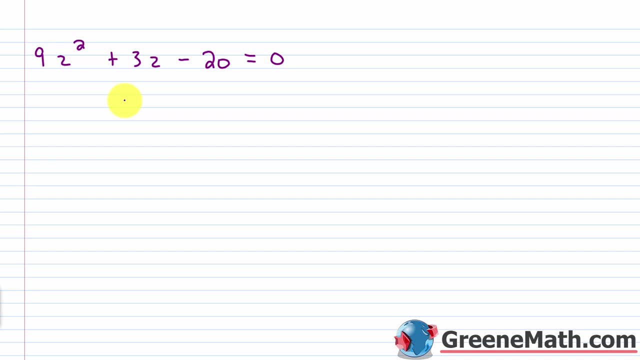 If we saw that, we know how to solve it. It's a quadratic equation, So we can use our quadratic formula. We can complete the square, You know, etc. etc. So if we think about what is a, That's 9.. That's the coefficient for the squared variable. 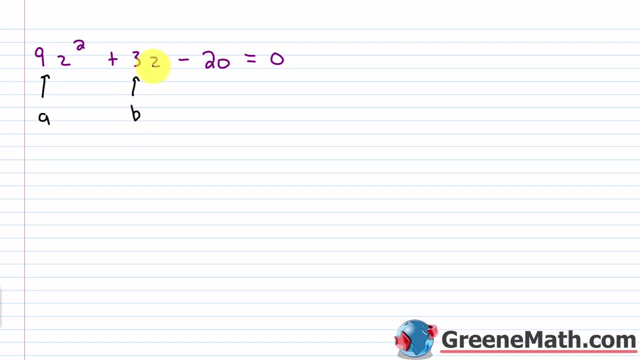 This is a, What's b? That's 3.. That's the coefficient for the variable raised to the first power. And what's c? C is going to be negative 20.. That's your constant, So the quadratic formula, in case you forgot. 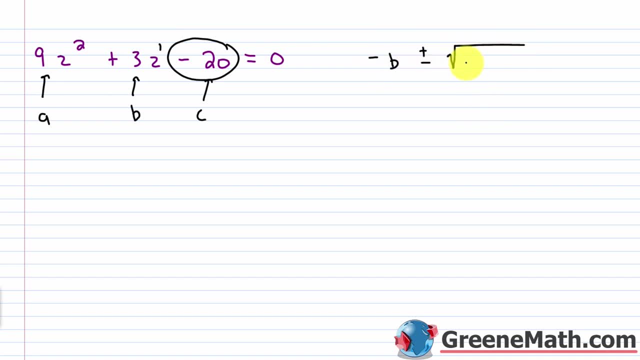 It's negative b plus or minus the square root of b, squared minus 4ac, all over 2a. So we're just going to plug in Right. So we know that b is going to be 3.. So I'd have negative 3.. 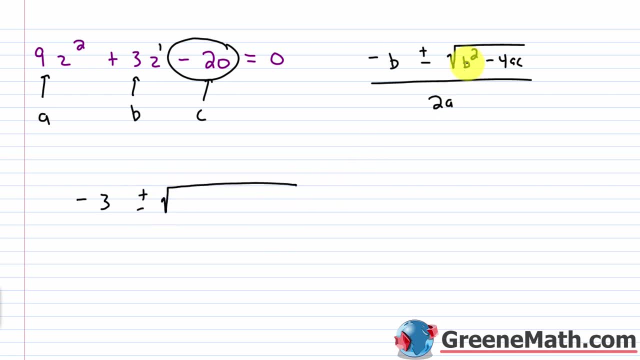 And then plus or minus the square root of b. squared Again, b is 3.. So 3 squared is 9.. Minus 4 times what's a, a in this case, is 9.. Then times c, c in this case is 9.. 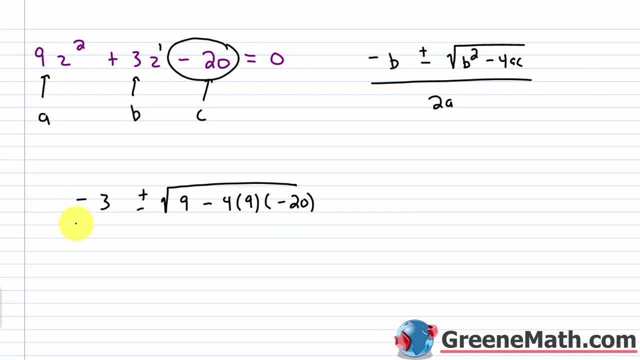 9. 9.. c in this case is negative 20. This is all over 2 times a. Again, a is 9.. So 2 times 9 is 18.. So I forgot to put z equals. Let me put that over here. 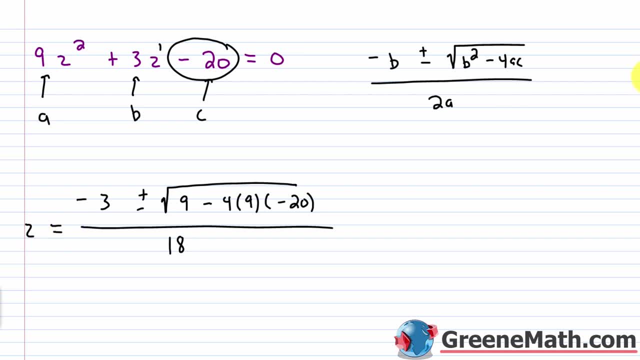 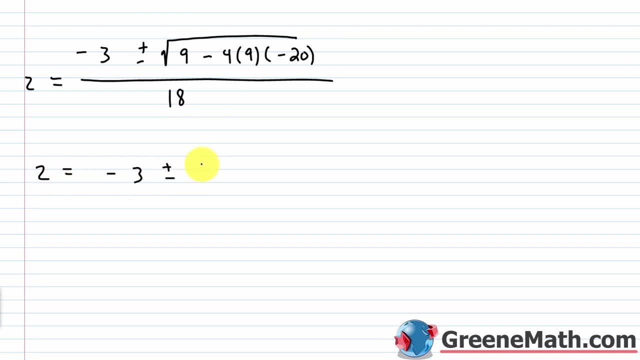 Z equals this: Scroll down, Get a little room going. So we'd have: z is equal to negative 3 plus or minus the square root of 9.. And then I'm going to treat this as negative 4.. So negative 4 times 9 is negative 36.. 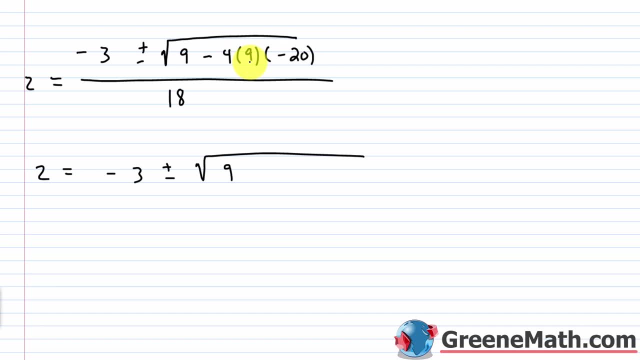 So when you take this here, 36 and then negative, 36 times negative, 20 is 720. So that would be positive 720. So I'd be adding 9 plus 720. And really we could just do this right now and say this is 729.. Okay, And this is over. 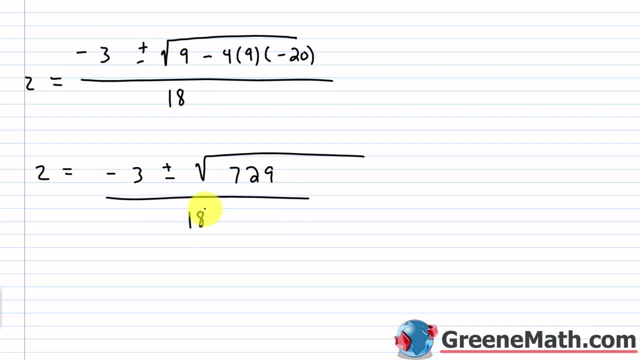 18.. Now the square root of 729 is 27.. So we'll say Z is equal to negative, 3 plus or minus. Again, this whole thing is going to simplify to 27 over 18.. So that's going to give us two different. 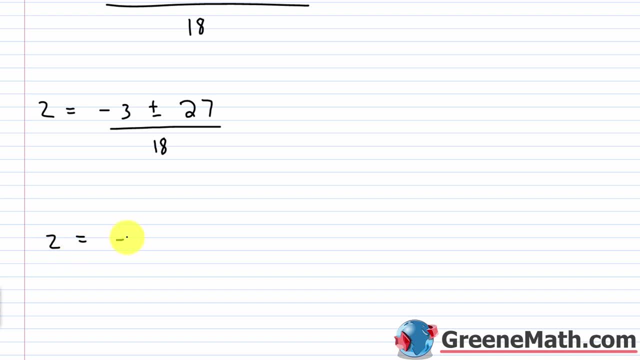 solutions. So we'll say that Z is equal to negative 3 plus 27 over 18.. And then, or Z is equal to negative 3 minus 27 over 18.. Let's scroll down a little bit more: Z is equal to negative 3 plus. 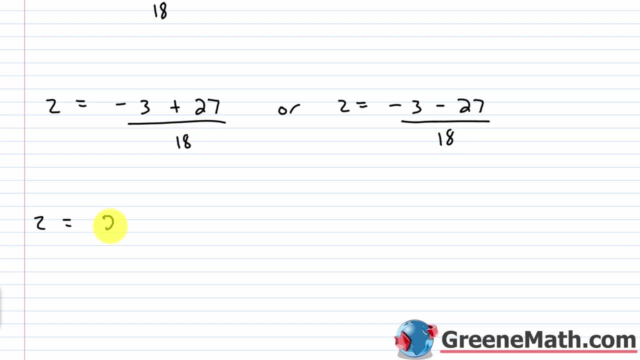 27 is going to be 24.. So you'd have 24 over 18.. Each is divisible by 6.. 24 divided by 6 is going to be 4.. 18 divided by 6 is going to be 3.. That's going to give us four thirds. Then, or over here, negative 3 minus 27. 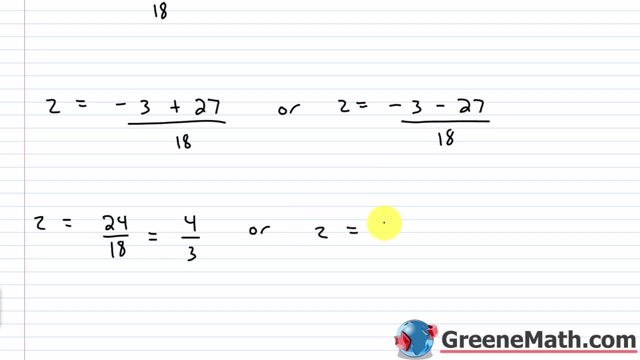 is going to be negative 30. So Z is equal to negative 30 over 18.. Each of these is going to be divisible by 6. So negative 30 divided by 6 is negative 5. And then 18 divided by 6 is: 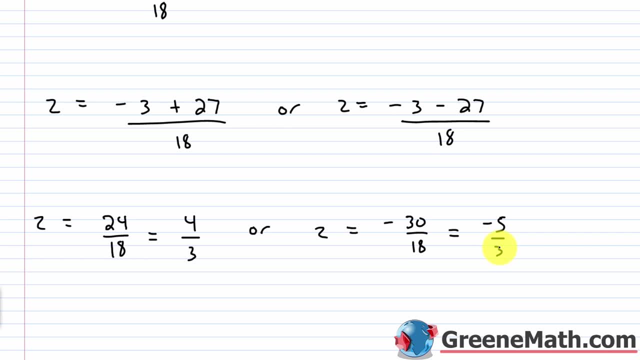 30. So Z could be four thirds or Z could be negative five thirds. Now let's stop for a minute. A lot of people make it to this point and they stop and they hand in their test or they finish the problem and they say: I'm done, You're not done, You're not solving for Z. 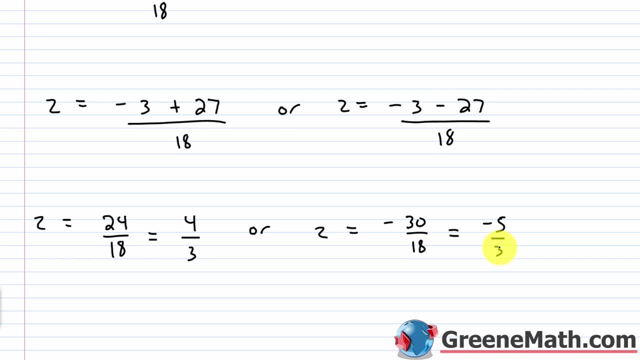 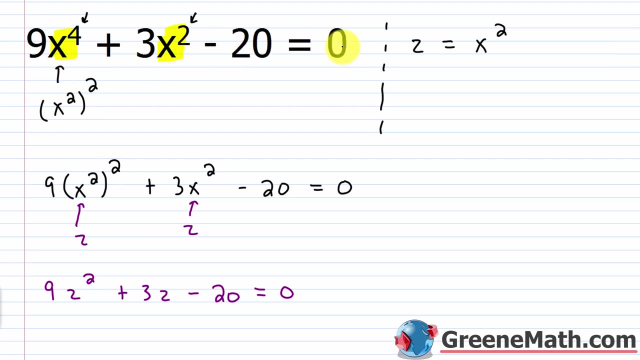 You're solving for X. You remember, if we go all the way back up here, our original problem was 9X to the fourth power plus 3X, squared minus 20 equals zero. So I still don't know what X is. I. 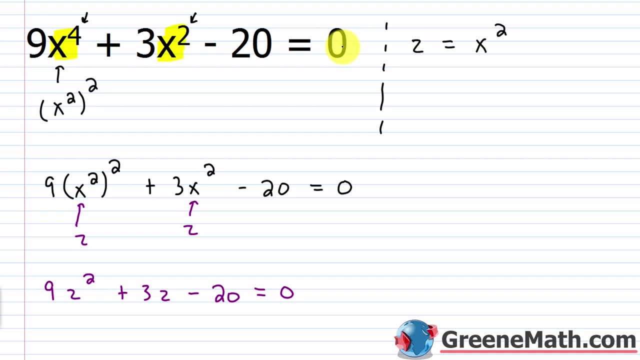 just know what Z is, and Z equals X squared. So I've got to substitute again And a lot of people just think, oh my, it's a lot of work. It's kind of a tedious process but it is simple. So we found: 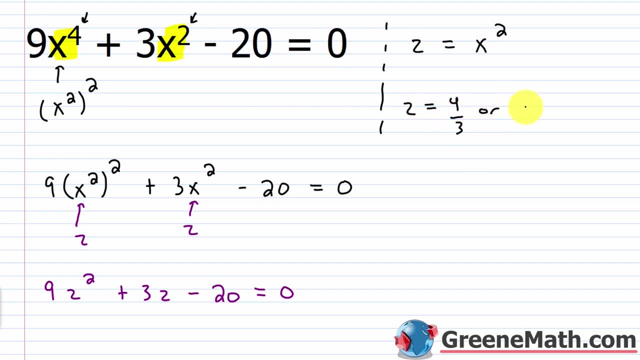 that Z was equal to four thirds or Z was equal to negative five thirds. So let me erase all this real quick. I don't need it anymore. And since Z equals X squared, I can simply say X squared is equal to well, Z equals four thirds and X squared equals Z. 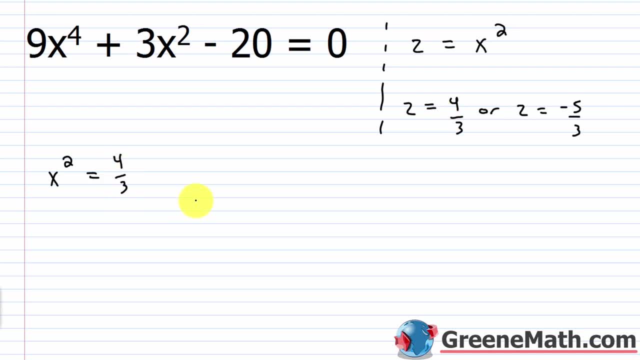 So X squared is equal to four thirds. Or again, Z is equal to negative five thirds. X squared equals Z. So I can say X squared is equal to negative five thirds. So I can solve this using the square root property. I can take the square root of this side, I can go plus or 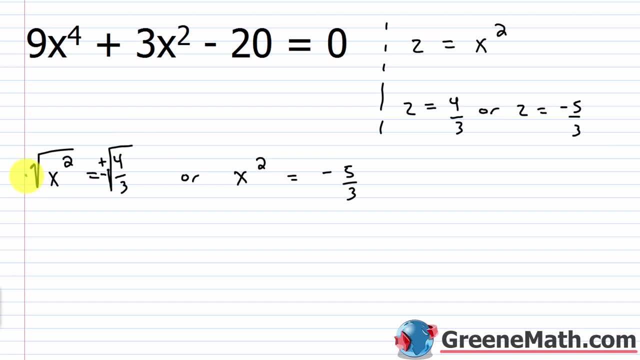 minus the square root of this side. So this would cancel here and I'd have X, And this is equal to plus or minus the square root of four over the square root of three. Let's just write it like that, So we know that the square root of four is two. So let's just go. 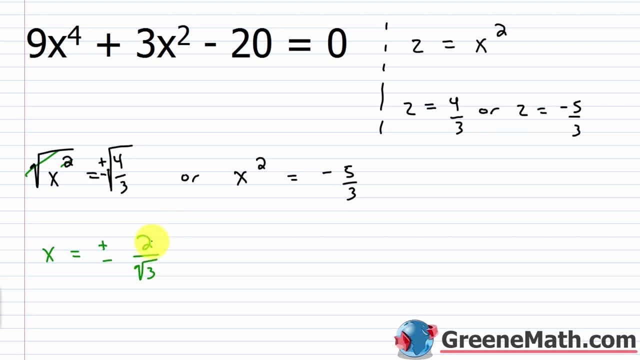 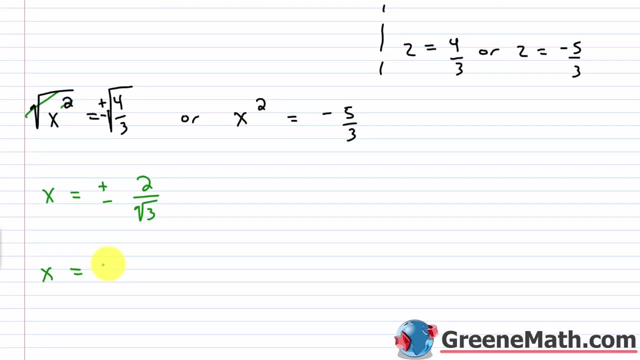 ahead and say this is plus or minus two over the square root of three, And of course we don't want a radical in the denominator. So we'll say this is X is equal to two over the square root of three, or X is equal to negative two over the square root of three. And if we rationalize the denominator, 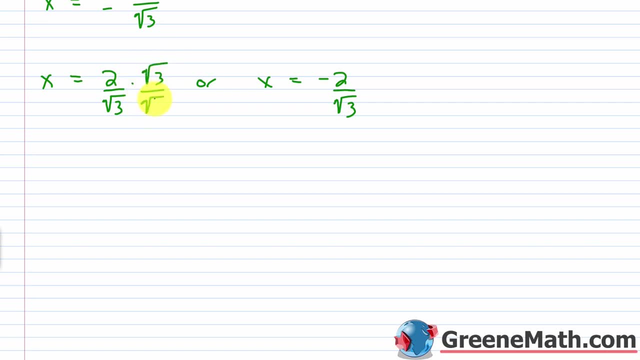 I multiply this by square root of three. I multiply this by square root of three, So I end up with: X is equal to two times square root of three over three, Or X is equal to, in this case, times square root of three over square root of three, negative, two times square. 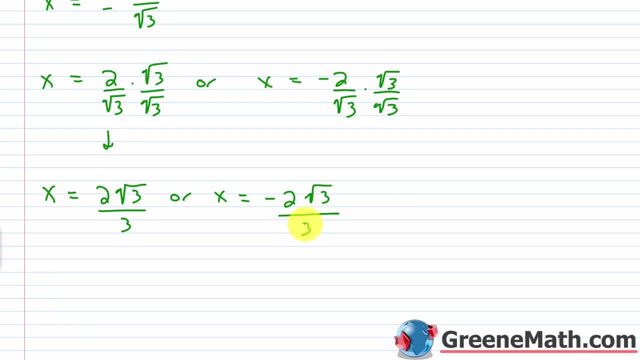 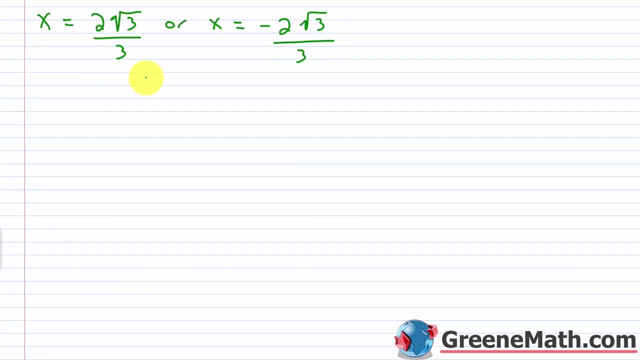 root of three over three. So that's one pair of solutions there. You've got another pair coming, So let's copy this and we're going to put this on the next sheet. Okay, So we'll just kind of leave that there for now. We'll go back up. So now we'll deal with the next pair of solutions. 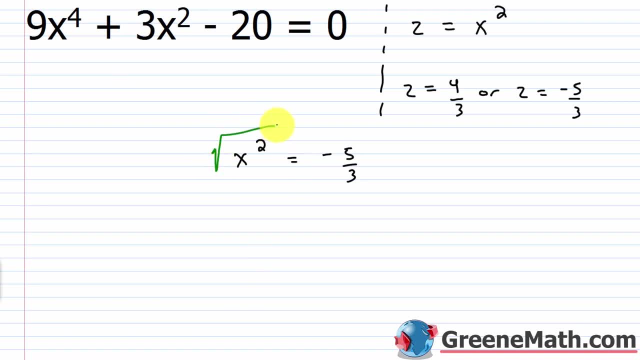 with this guy, x squared equals negative five thirds square root of this side, plus or minus the square root of this side. so this guy will cancel. with this guy I'll have: x is equal to plus or minus the square root of negative five over the square root of three. now the square root. 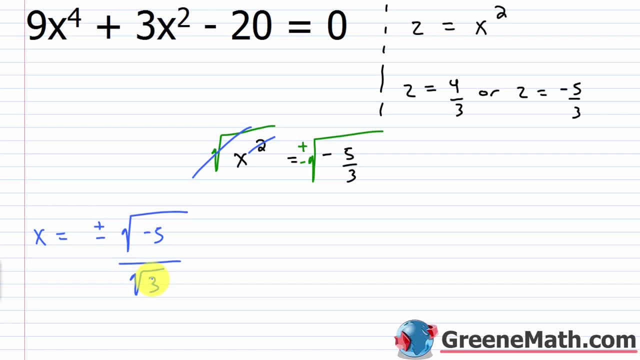 of negative five. of course I want to pull the negative out of that right, so I pull an i outside and I get rid of the negative and really the square root of three and the square root of five. I can't do anything with either one of those, so I just want to rationalize and I don't need to split. 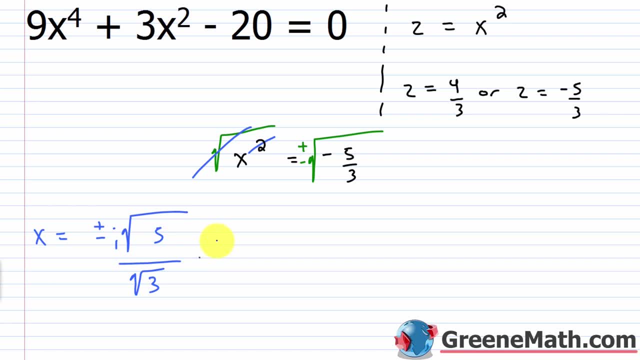 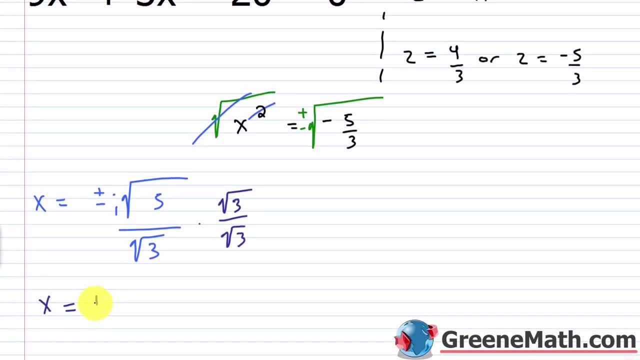 this into two different solutions. for now I can do that. when I get down there I'll say: this is times the square root of three over the square root of three, to rationalize. and so I'll say we have: x is equal to plus or minus. i times the square root of five times three, which is 15. 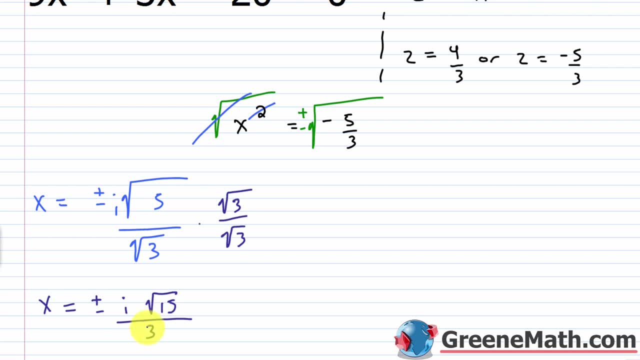 over square root of three times square root of three is three, so x equals plus or minus. i times the square root of 15 over three, so let's go down. let me copy this real quick and we'll turn this into two different solutions. we'll say: x is equal. 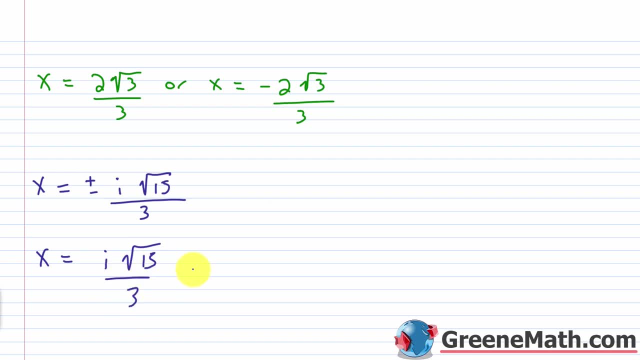 to: i times square root of 15 over three, or x is equal to negative, i times the square root of 15 over three. if you want to, you can do a solution set here and let me just kind of drag this up and I'll do one so you can see how you write that. let's use a more. 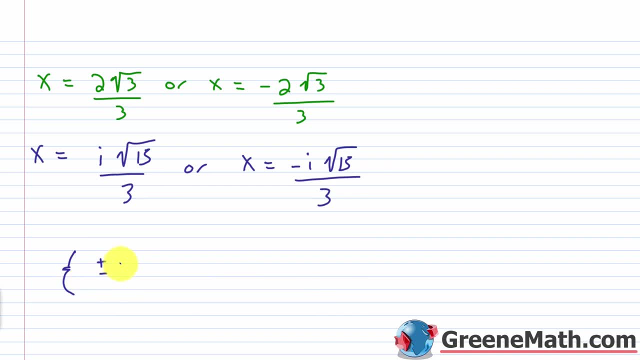 compact form, just make it easier. we'll put plus or minus two times the square root of three over three comma. we'll put plus or minus i times the square root of 15 over three. so those would be our two solutions. really it's four solutions. it's two times square root of three over three, negative two. 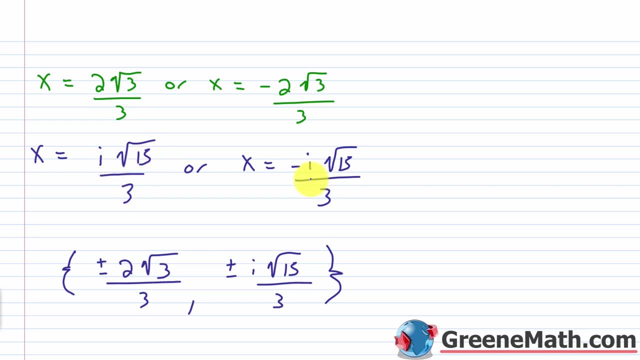 times square root of three over three, i times square root of 15 over three. or, finally, negative, i times square root of 15 over three. all right, let's take a look at another problem and we see that we have one that fits the same pattern we saw last time. 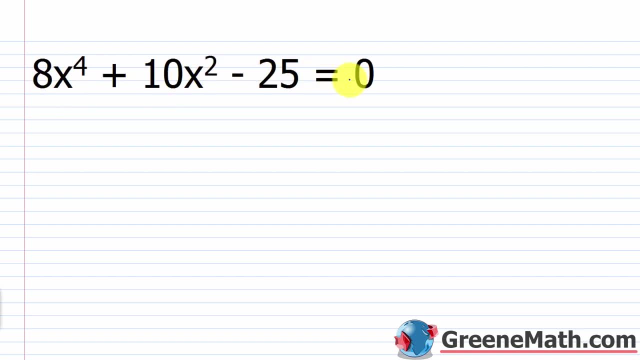 8x to the fourth, power plus 10x squared minus 25 equals zero. so again you've got three terms involved, just like you'd see, with ax squared plus bx plus c, then the next thing you're looking at is the larger exponent is a four, the smaller one is a two, so it's double, right, the four is doubled. 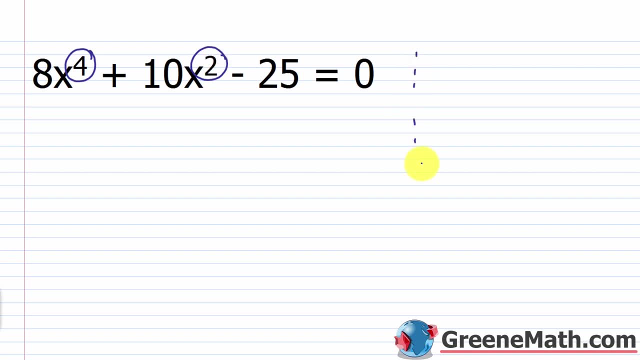 out of the two. so all I need to do to make this into a quadratic equation is make a substitution where, let's say, q is equal to the variable raised to the smaller power. so in that case this is x squared, and again you're going to have to rewrite this using your rules for exponents. 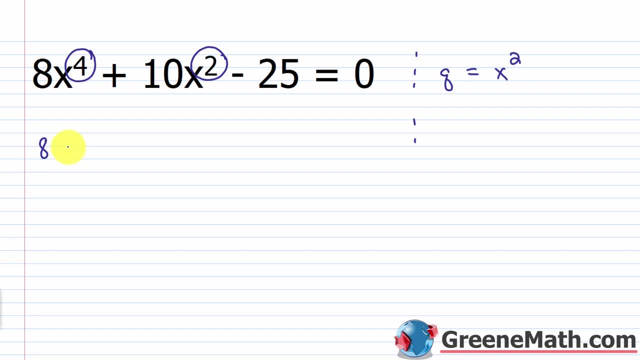 so that you can make that substitution. so I would say this is: 8x squared squared plus 10x squared minus 25 equals zero. I want to plug in a q. everywhere I see an x squared, and then it's very easy to do that. so I'm going to plug in a q and I'm going to plug in a q and I'm going to. 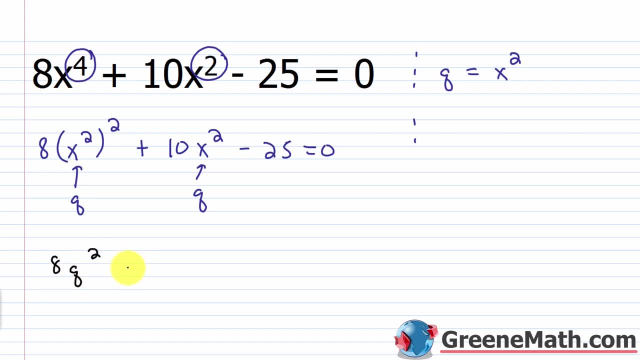 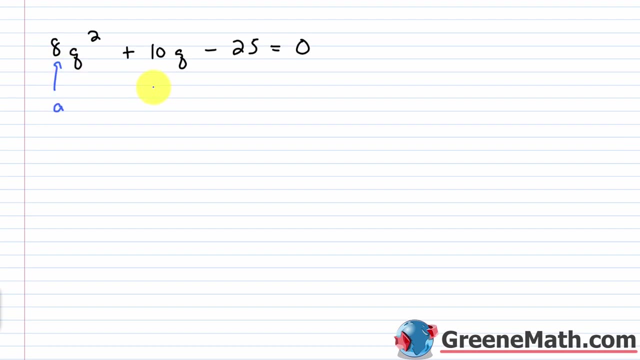 say this is 8q squared plus 10q minus 25 equals zero. all right, so we can again solve this using the quadratic formula. I know what my a, b and c are here. this is of course a, this is my b, and negative 25 is my c. so we want again for the quadratic formula: negative b plus or minus. 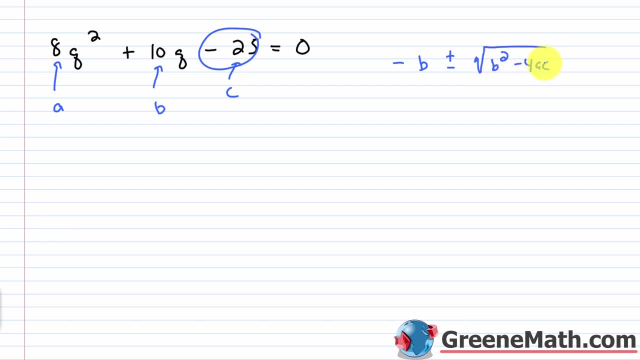 the square root of b squared minus 25 equals zero. so we can again solve this using the quadratic formula. I know what my a, b and c are here. this is my b and c are here. this is my b and c are here, plus or minus. the square root of b squared again b is 10. so 10 squared is 100 minus 4 times for a. 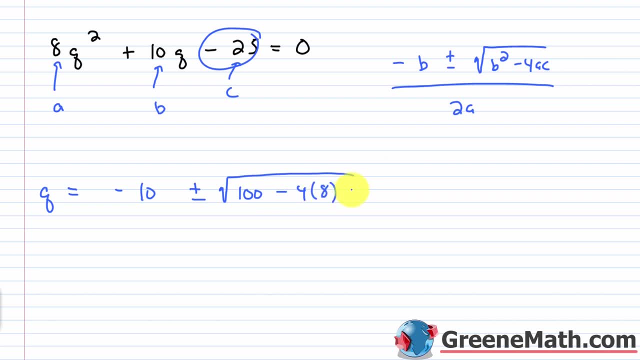 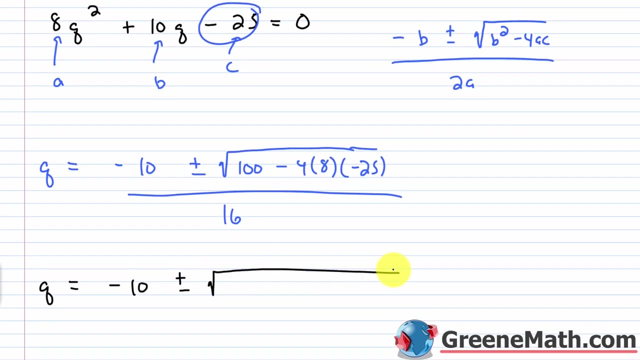 it's 8. for c it's negative 25. so times negative 25. and then this guy is all over. 2a is 8, so 2 times 8 is 16. so q is equal to negative 10 plus or minus the square root of you've got 100. 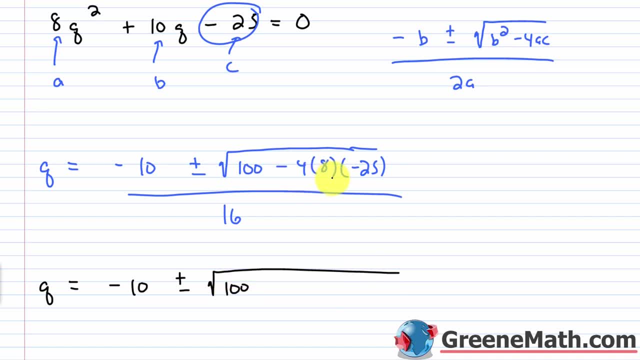 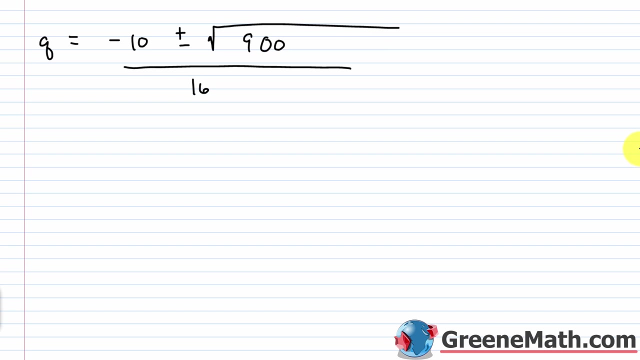 sitting out in front. you basically have negative 4 times 8, that's negative 32, and then negative 32 times negative. 25 is 800. so you'd have 100 plus 800, which would be 900. so then this is all over. so let's scroll down and get some room going here. so to finish this up, we have: q is equal to. 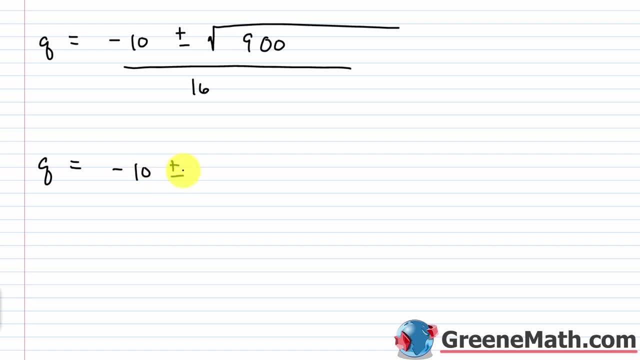 you have negative 10 plus or minus. the square root of 900 is 30. this is over 60. so two different solutions we're going to get here. let's go ahead and draw those out real quick. you have: q is equal to negative 10 plus 30. so negative 10 plus 30 over 16. 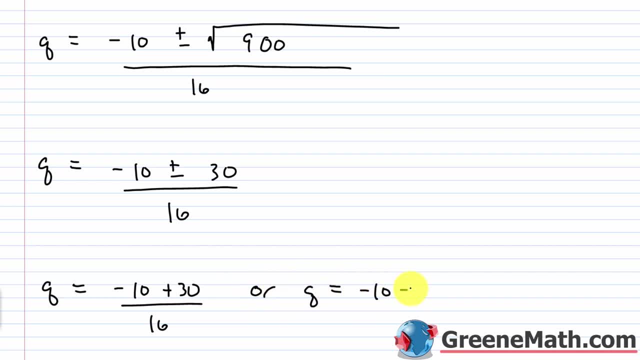 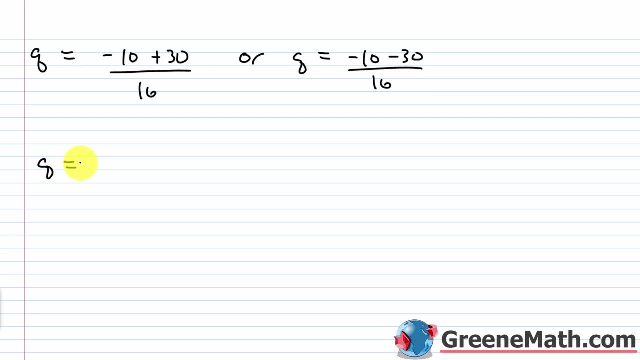 or q is equal to negative 10 minus 30 over 16.. okay, so for the first one here, q is equal to negative. 10 plus 30 is 20, so you'd have 20 over 16. each is divisible by 4, but if i 20 by 4, i get 5. 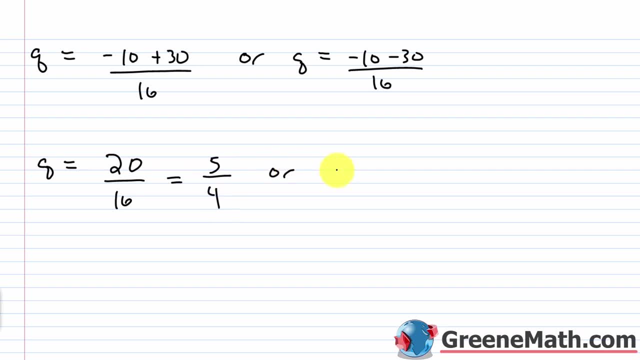 16 divided by 4 is 4 then. or you'd have: q is equal to negative. 10 minus 30 is negative 40. so negative 40 over 16 each here is going to be divisible by 8. negative 40 divided by 8 is going to be negative 5. 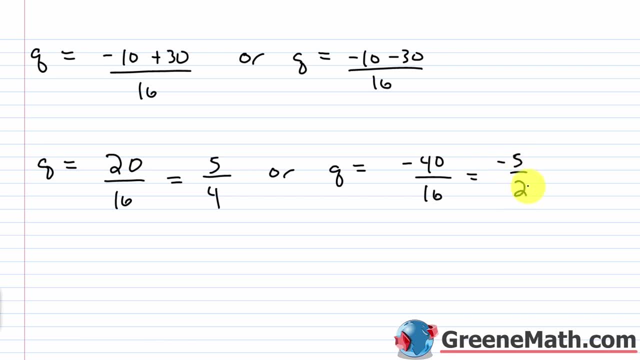 16 divided by 8 is going to be 2, so you end up with negative 5 halves there. so you've got q equals 5 fourths, or q equals negative 5 halves. again, we're not done right. we made a substitution to solve this using the quadratic formula, so we've got to go back and substitute again. 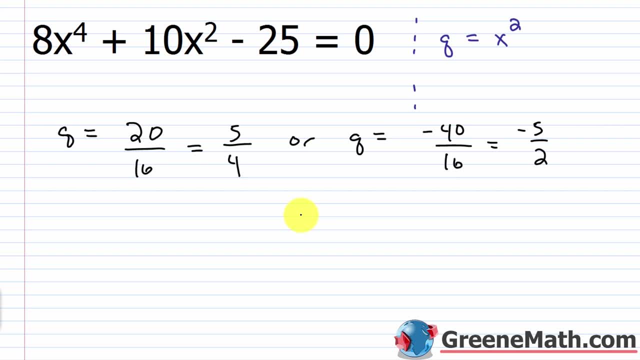 and then we can get our answer all right. so we come back to our original problem, which was the 8x to the fourth power plus 10x squared minus 25 equals 0. so again we substituted for x squared, we said q equals x squared. we found out that q was 5 fourths, or q was negative, 5 halves. so 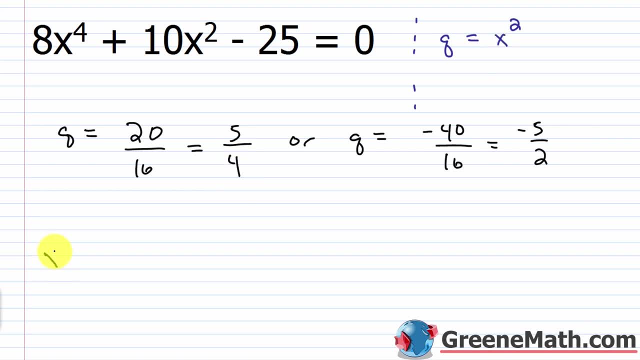 i can say that x squared equals 5 fourths, or x squared is equal to negative 5 halves. so let's scroll down a little bit. so i'm going to solve this by taking the square root of each side. so if i take the square root of this side, 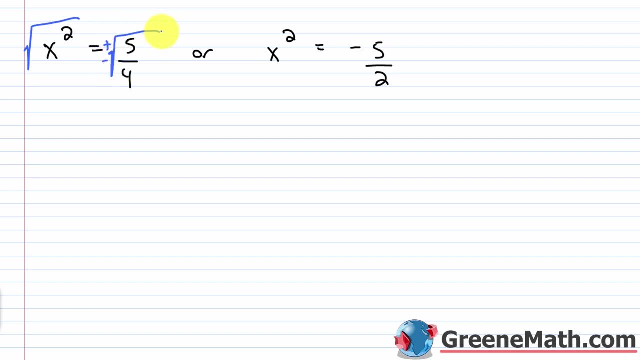 and i say plus or minus the square root of this side. so i would have: x is equal to plus or minus the square root of 5 over 2. then, coming over here to deal with this one, i have x squared equals negative 5 halves. so i would take the square root of this side and then plus or minus the square. 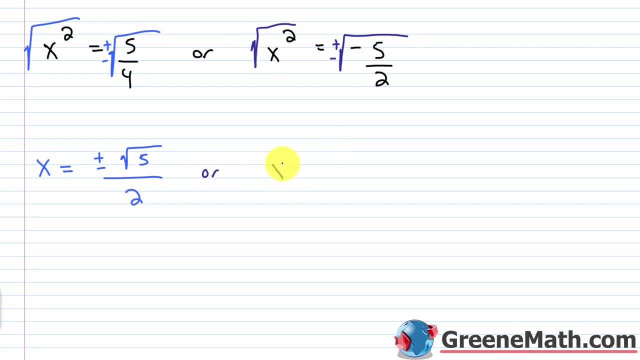 root of this side. so we know that this would be: or x is equal to. i'd have plus or minus the square root of negative 5 over the square root of 2. this one's a little harder to clean up because i have that square root of 2 down there, so i'm going to have to rationalize the denominator and then also. 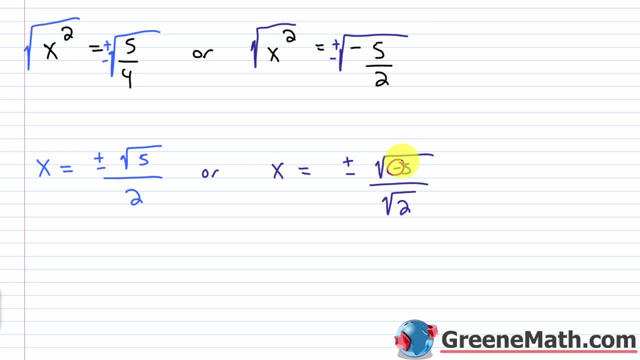 i have a negative radicand, so for this one i could just say that x is equal to plus or minus. i know that would come out as i right that negative there. so i times the square root of 5 over the square root of 2 and then, to rationalize, i could multiply by the square root of 2. 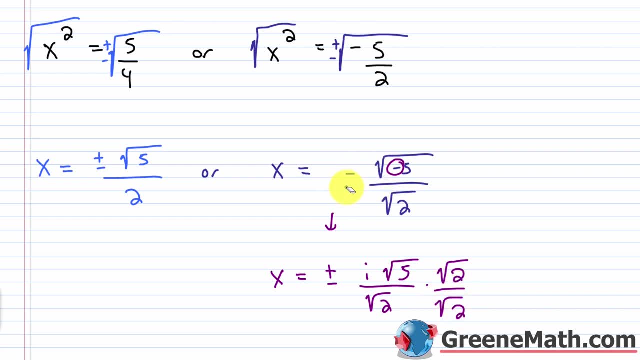 over the square root of 2, and let me just write this up here. what i'd end up with is that x is equal to plus or minus. i times the square root of 5. times square root of 2 is the square root of 10. 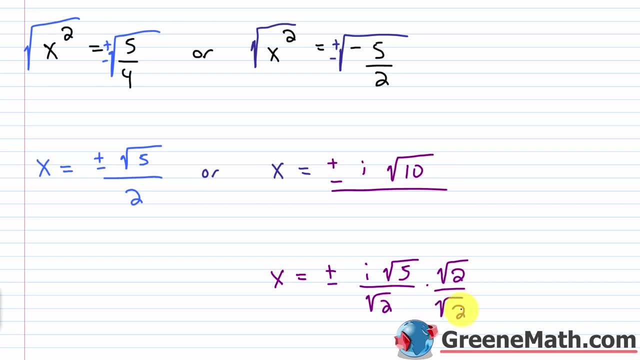 over. you have square root of 2 times square root of 2, which is 2. let me erase this, let me kind of write that a little better. so again, we had plus or minus. i times the square root of 10. this is all over 2. 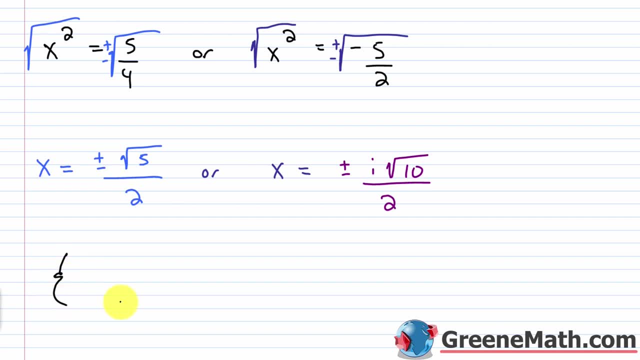 you can always write this in a solution set. so let's say in solution set notation: we have plus or minus the square root of 5 over 2 comma. we have plus or minus, i times, the square root of 10 over 2, and again, this is four different solutions. you have: x equals square root of 5 over. 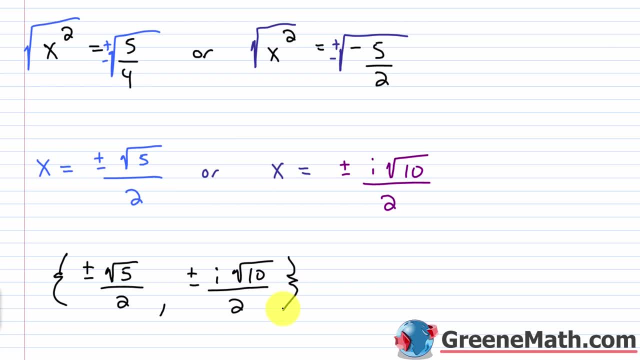 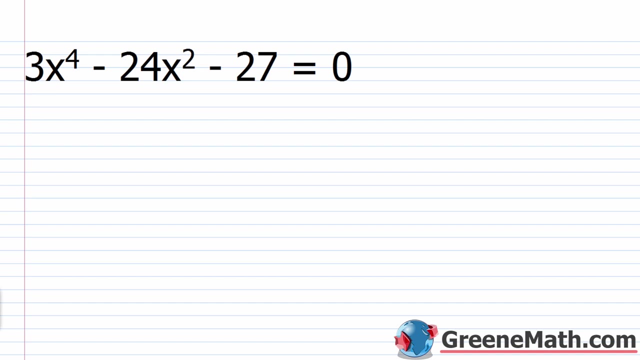 2. you have x equals negative square root of 5 over 2. you have x equals i times square root of 10 over 2. and then you have x equals negative i times square root of 10 over 2. so let's take a look at another one. we have 3x to the fourth power minus 24x squared minus 27. 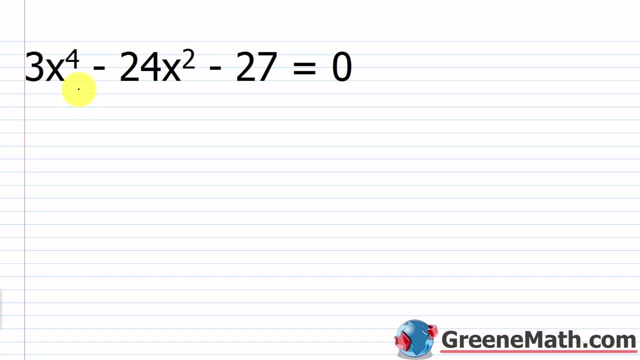 equals zero. so again you see that you have three terms and you have your pattern where you have a constant. you have x raised to a smaller power. you have x raised to a larger power, that the larger power is double that of the smaller power. right, four is double that of two and you're going to 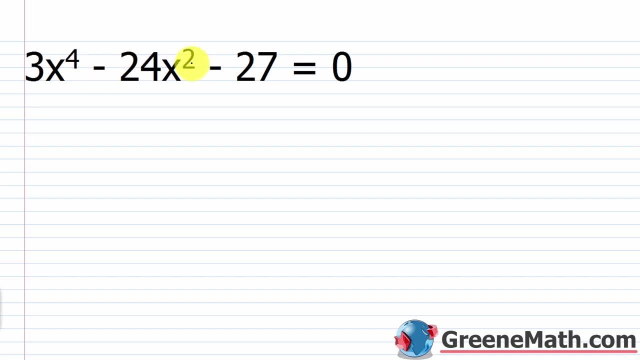 see examples where you have x to the sixth power and x to the fourth power, and you're going to see examples where you have x to the fifth power and x to the sixth power. and you're going to see examples where you have x to the sixth power and x to the seventh power, and you're going to see. 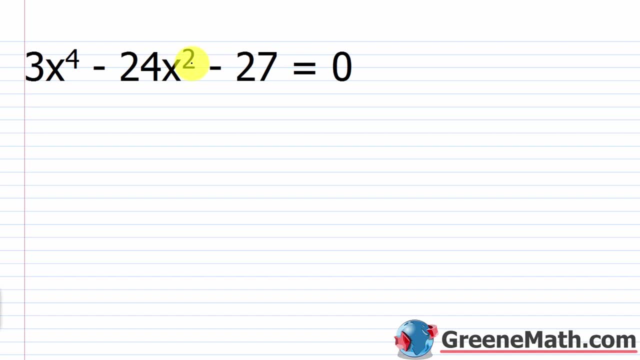 where you might see x to the 18th power and x to the ninth power, right? so you're just looking for this guy right here to be twice this guy right here, okay, the larger to be double that of the smaller. so when i want to make my substitution here, let's just use u, let's say let u be equal to. 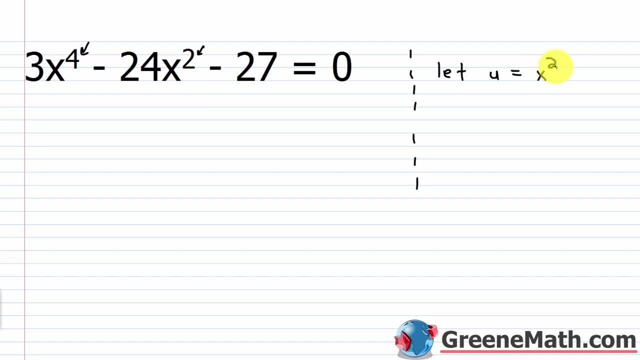 x squared. so i'm going to plug in a u. everywhere i see an x squared. but again i've got a kind of transform, transform. transform this a little bit so it makes it easier for me to visualize what's going on. I'm going to write: 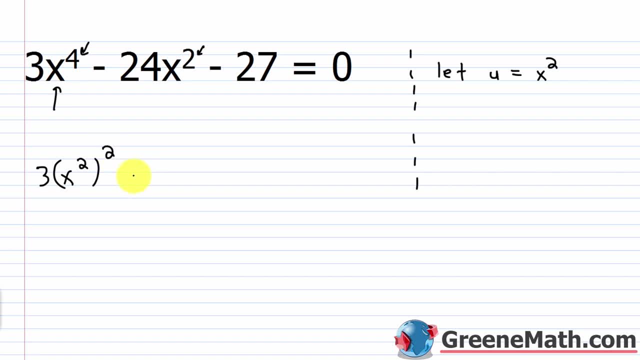 this as 3x squared, squared minus 24x squared minus 27 equals 0.. Plug in a? u here and here, So that gives me 3u squared minus 24u minus 27 equals 0.. All right, So now we know we have a. 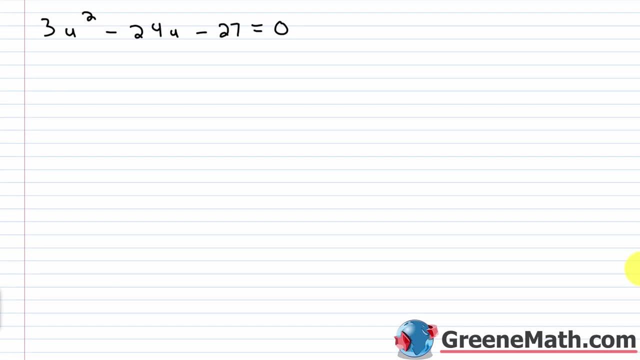 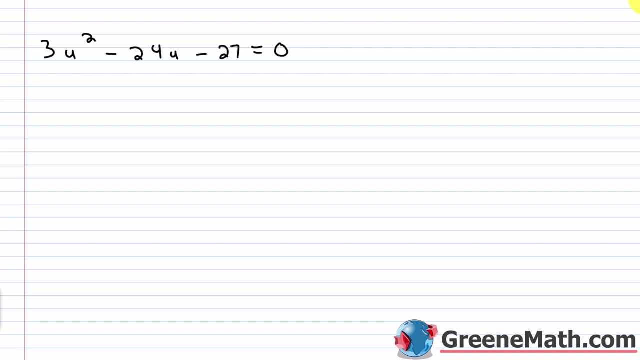 quadratic equation and very, very easy to solve. at this point, If you look, you can see that right away you could factor a 3 out and you could solve this with factoring Right. So I could pull a 3 out and I'd have u squared minus 8u minus 9, and this is equal to 0.. Now, because this is an equation, 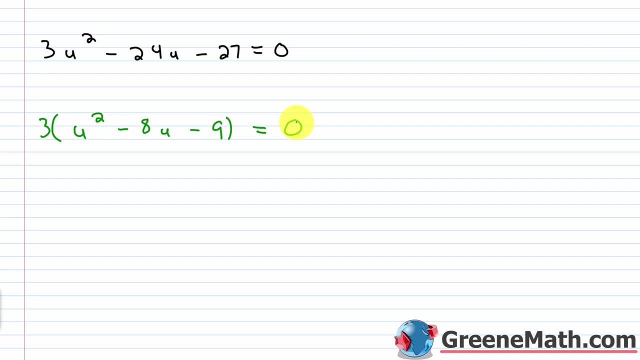 I can divide both sides by the same non-zero number and I'm not changing the solution. So I can divide both sides here by 3, and 0 divided by 3 is still 0. So really I'm just kind of reducing some of the tediousness of the problem because I'm working with smaller numbers. 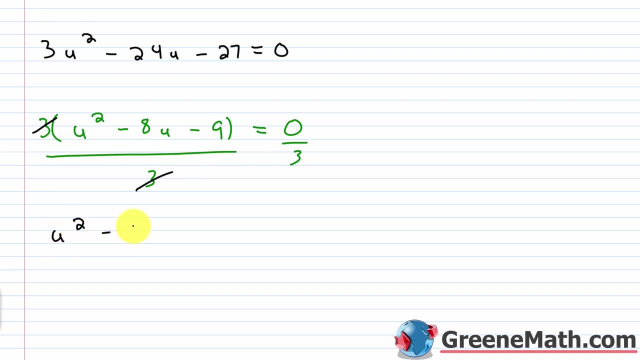 Right, So it's just something you want to do. So this is: u squared minus 8u minus 9 equals 0.. And I can solve this using factoring pretty easily. Give me two integers whose sum is negative 8 and whose product is negative 9.. 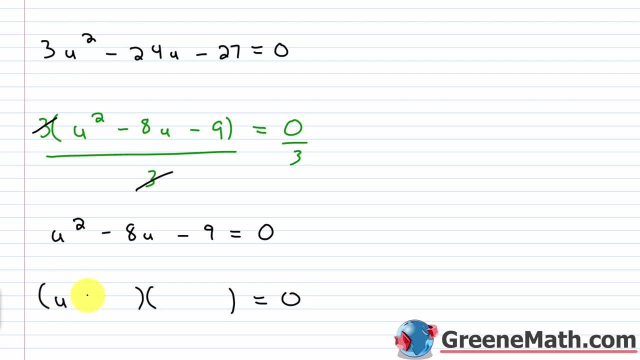 Well, that's negative 9 and positive 1.. So u minus 9 and then u plus 1.. So the solutions: I know that I would set this up to be u minus 9 equals 0 or u plus 1 equals 0. And of course, I add 9 to. 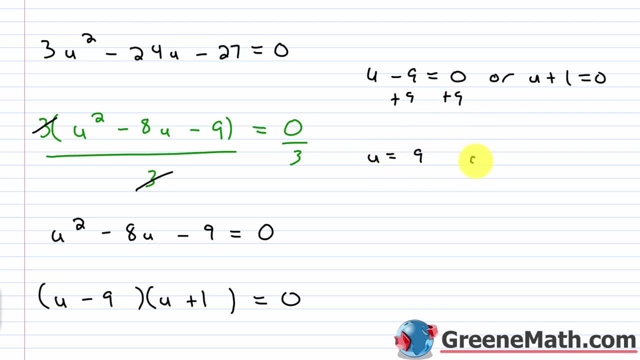 both sides of the equation- here I get- u equals 9.. Then, or I subtract 1 away, each side- here I get u is equal to negative 1.. So let's copy this, All right, So we know that u equals 9 or u equals negative 1.. But again we got. 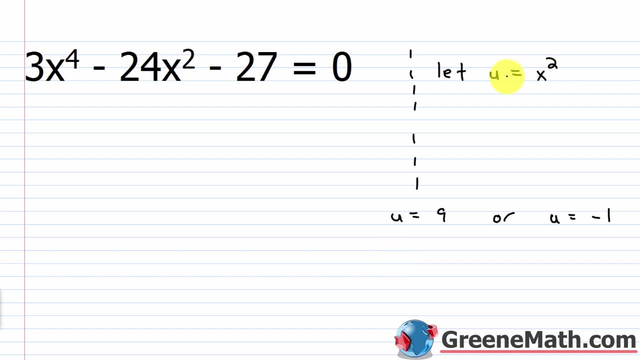 to find out what x is. So if x squared equals u and u is 9, then x squared really equals 9.. Or u also equals negative 1.. So x squared also equals negative 1.. So to find x, let's take the. 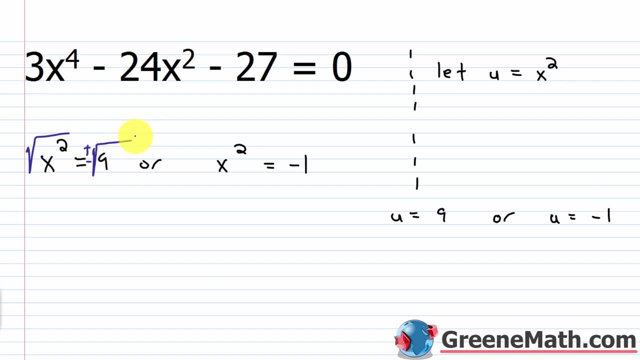 square root of each side over here, And so I would have x squared minus 9.. And so I would have x squared equal to plus or minus the square root of 9.. The square root of 9 is 3.. So x equals positive 3 or. 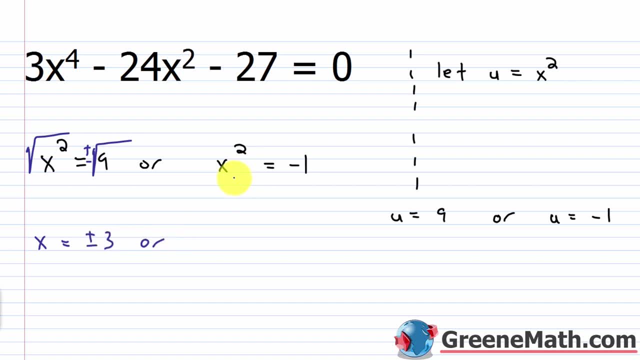 negative 3.. Then or you have take the square root of each side over here And you would have: x is equal to plus or minus. the square root of negative 1 is known as i right by definition. So plus or minus i. So pretty simple for this one In solution set notation we would just say plus or minus 3.. 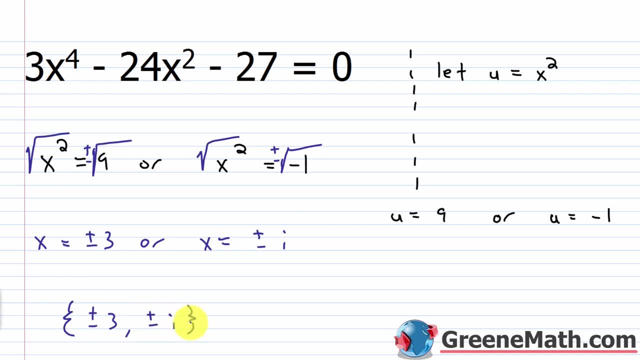 Comma plus or minus i. Again, you've got four solutions there. You've got: x can be positive, 3. X can be negative, 3. X can be positive, i, X can be negative, i. All right, Let's wrap up the lesson. 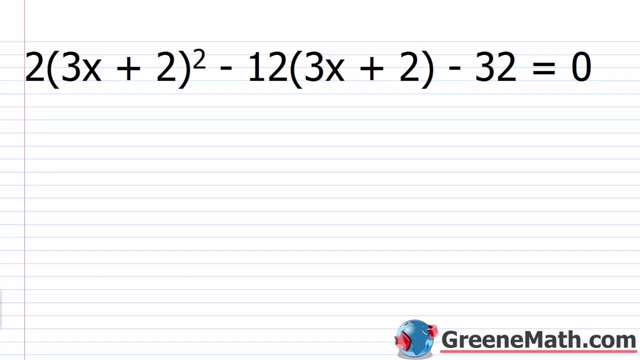 with one that's a little bit different. So you have 2 times the quantity 3x plus 2 squared minus 12 times the quantity 3x plus 2 minus 32 equals 0. So most of the problems you encounter when you're working on this topic are going to be pretty straightforward, like the ones we looked at. 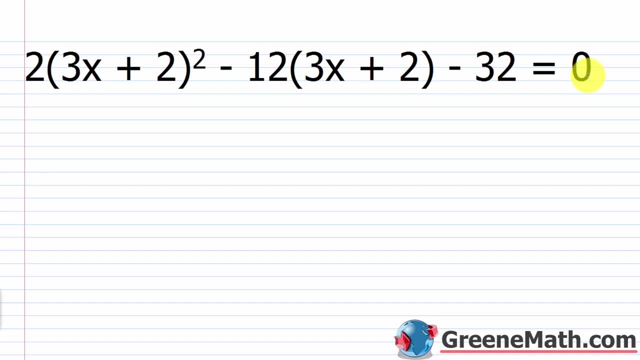 You might get some variations where you have x to the 6th power and x cubed. Or you might get again x to the 18th power, x to the 9th power. Again, you're looking for that higher power to be double that of the small. Okay, that's what you're looking for Here. it's not quite so obvious. 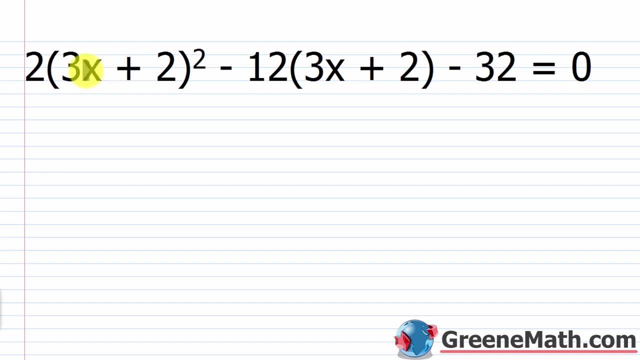 but if you just think about this, right here I have 3x plus 2 and 3x plus 2.. I have an exponent that's 2 and an exponent here that's really a 1.. So the 2 is double that of the 1.. So that's. 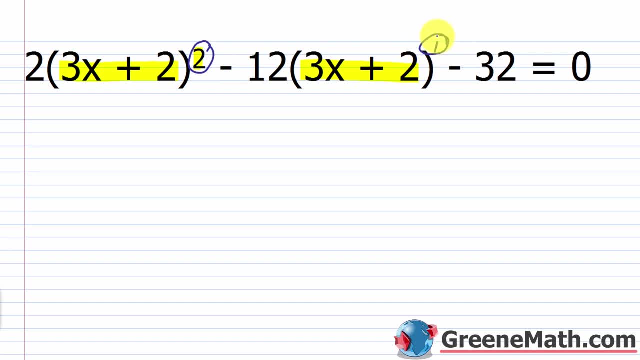 1. Okay, If I made a substitution, If I said: let's let g. Okay, let's let g be equal to this quantity, 3x plus 2. Well, I'd plug in a g there and a g there, I'd have a quadratic equation. 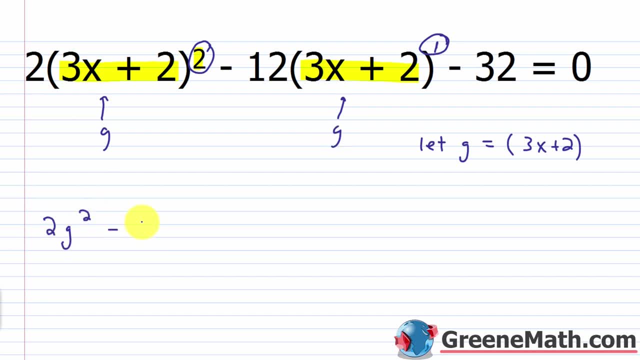 I would have: 2g squared minus 12g minus 32 is equal to 0.. Okay, pretty straightforward Now, with this guy right here, I have a common factor of 2.. So, again, to make this easy on myself, I can divide both sides of the equation by 2.. I can factor out a 2 and divide. 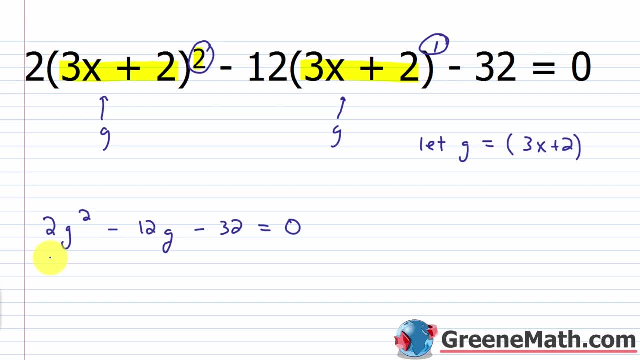 both sides of the equation by 2.. However, it's more comfortable for you Or you can work with it as it is. But again, if you can do something to make the number smaller, it always makes your calculations faster, Especially if you don't have a calculator. So let me just go through and divide. 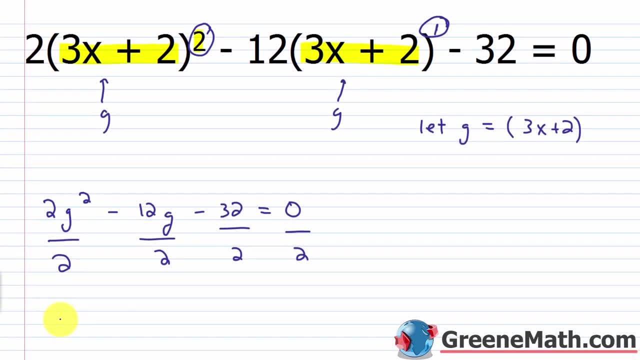 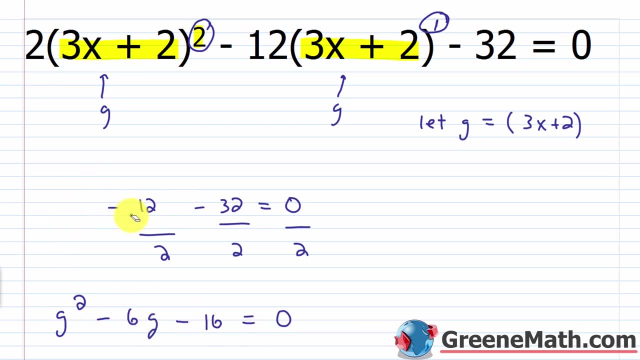 everything by 2.. I would have g squared minus 6g minus 16 equals 0.. All right, so let's erase this And I'm going to scooch this up here so we have some room, And can I factor? this guy Looks like I can, So give me. 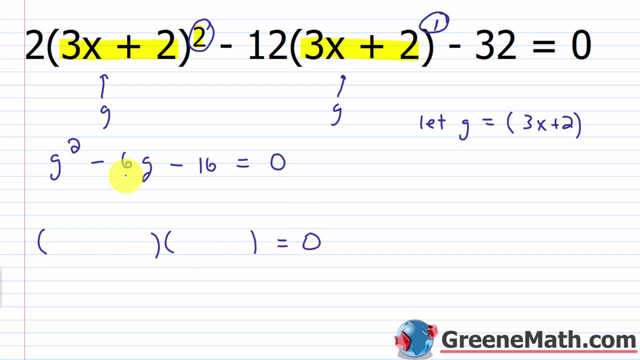 two integers whose sum is negative 6 and whose product is negative 16.. Well, I could do: negative 8 and positive 2. So g minus 8 and g plus 2.. Okay, so we all know at this point that g could be 8 or g could be negative 2. But again, 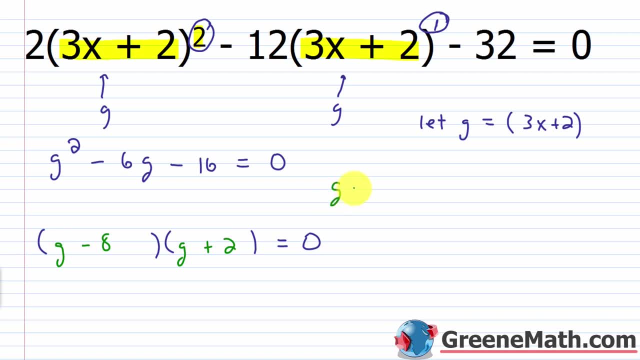 for completeness, we would say: g minus 8 equals 0, or g plus 2 equals 0.. Add 8 to both sides of the equation: here g equals 8.. Then, or subtract 2 away from each side of the equation: here g equals. 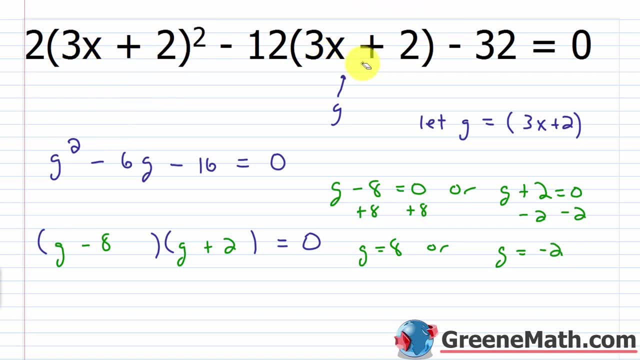 negative 2.. Let's erase all this real quick. Let's erase this. I'm just going to keep my solutions Now. we said that g was equal to, or g is the same as only 3x plus 2. So I can say that g equals 8.. 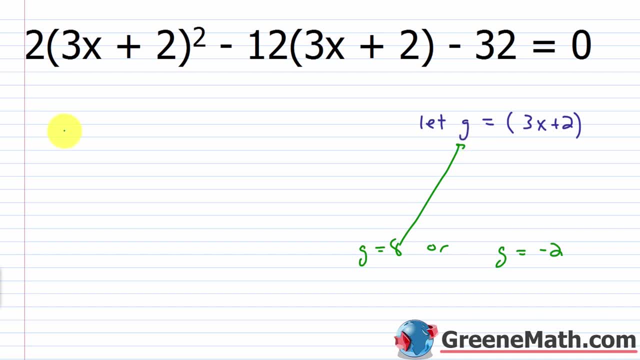 I can plug 8 in here and I can just say that 8 equal to or the same as the quantity 3x plus 2.. We now know how to solve this. This is very, very simple. Subtract 2 from both side de CEO apresent. 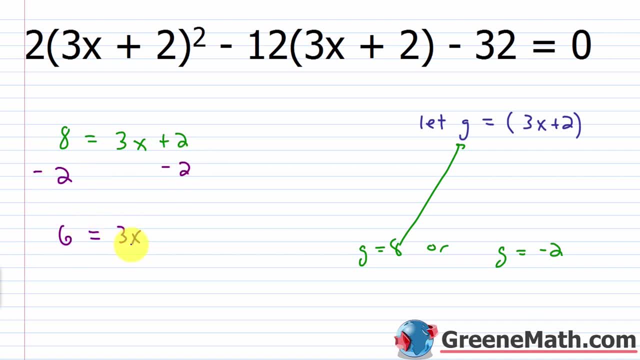 each side, you would have: 6 is equal to 3x. divide both sides by 3, and you would get that 2 is equal to x or x equals 2,. however you want to think about that, Then you can do the same thing. 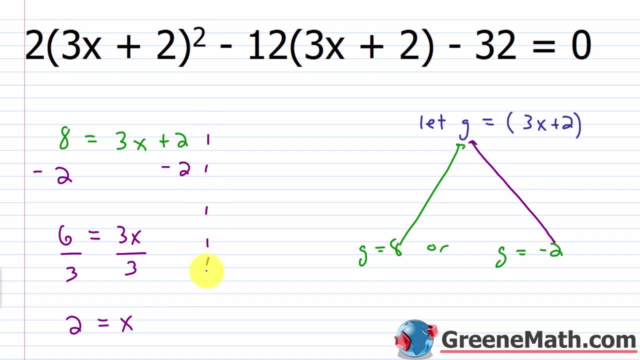 Plug in a negative 2 for g there and you would say that this is: OR. negative 2 is equal to 3x plus 2, subtract 2 away from each side of the equation, you would have that negative 4 is equal to 3x. divide both sides of the equation by 3, and you would say OR. 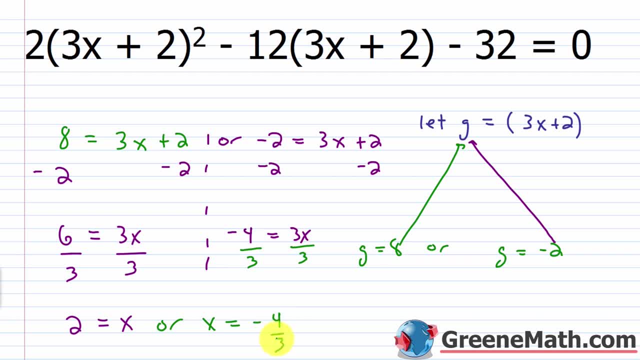 x is equal to negative 4 thirds. So x here is 2, or x is negative 4 thirds. let me put x on the left side, because that's how I like it and, of course, if you wanted to use a solution set, you could say negative. 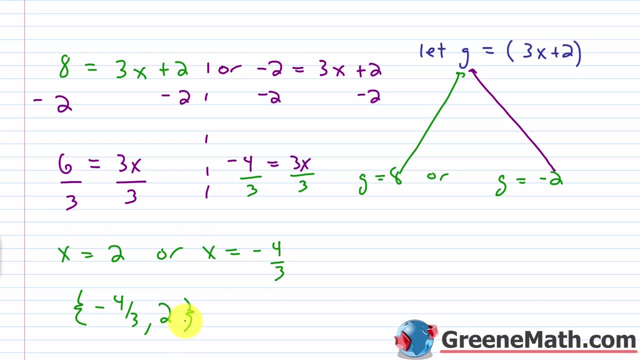 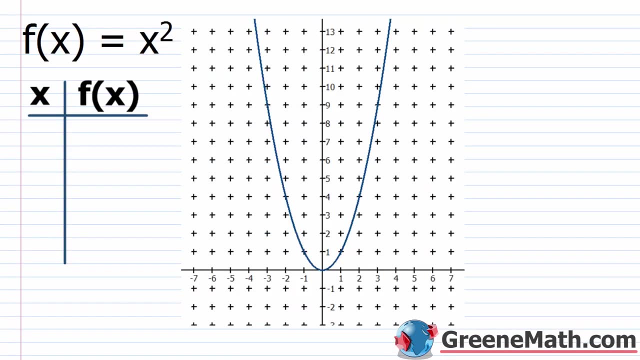 4 thirds, comma 2.. Hello and welcome to Algebra 2. Less Than 65.. In this lesson we're going to learn about graphing parabolas. So up to this point we've only graphed lines. As we move forward in math, we must be prepared to deal with more complex shapes. 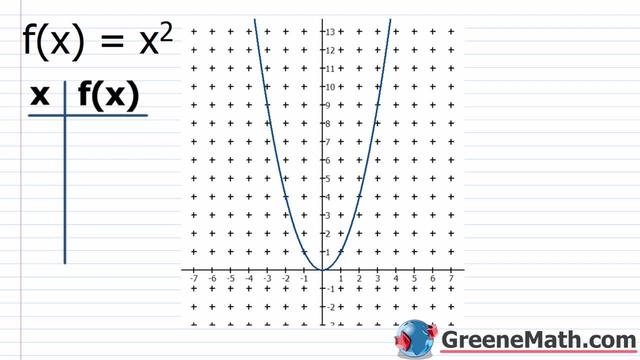 So the focus of today's lesson is to learn about something known as parabolas. Now, first and foremost, the graph of any quadratic function, or you could say the graph of any quadratic equation, is known as a parabola. So what we're going to start out today with is this: f of x equals x squared. 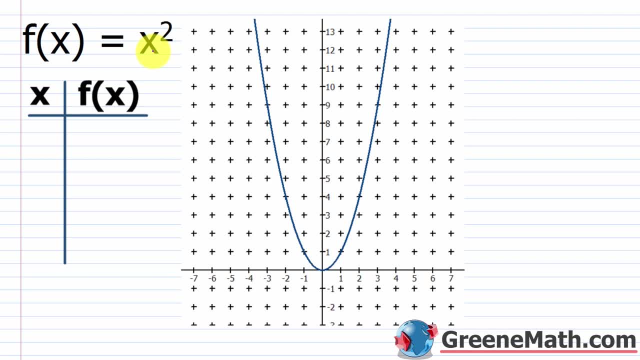 If this is generally what you're going to see in your textbook or in your class. this is going to be the first parabola you deal with and it's what we're going to use as a comparison when we're talking about shifts, and we're going to get to that in a second. 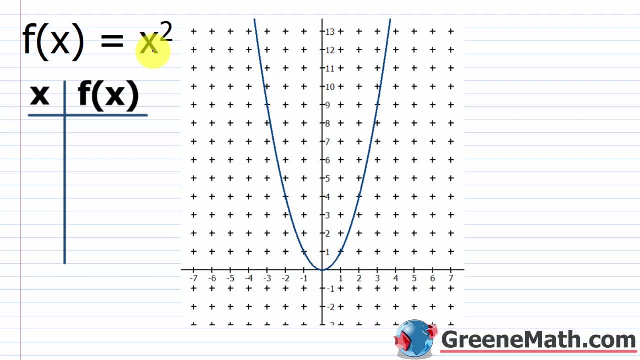 So what you'll notice about a parabola is that the shape kind of looks like a u, But depending on the function that you're given, this guy could be skinnier, it could be wider, it can open up as it does here, or it might also open down. 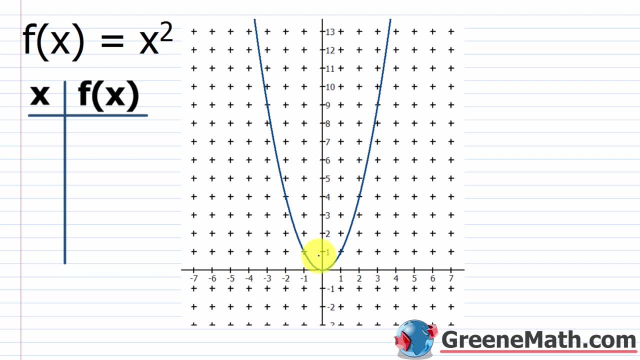 We're going to see examples of these not only in this lesson, but in a lot of other lessons, but in the next lesson where we continue talking about parabolas. Now, this function is already graphed for us, and you might say: well, why is that the case? 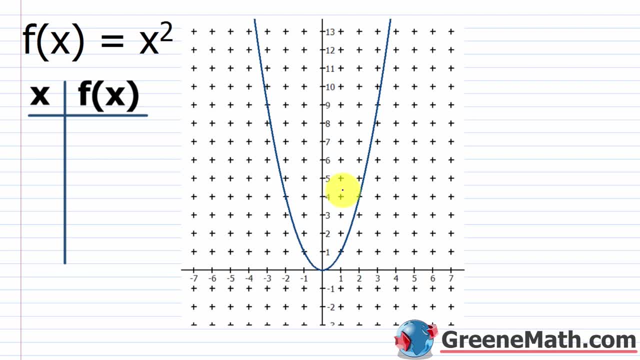 Well, we aren't really going to talk too much about how to sketch the graph of a parabola At this point. the process of graphing is pretty straightforward: You gather some points, you plot them and then you sketch. The one thing I want you to know is that the process of graphing something that's not linear. 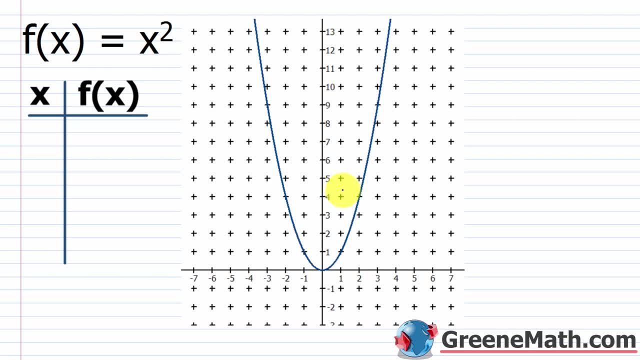 is a little bit more difficult. You're going to be less accurate And generally, if you want something that's going to be accurate, you either need to use a graphing calculator or some type of graphing software. So to eliminate the inaccuracies. I just have the curve already sketched for us. 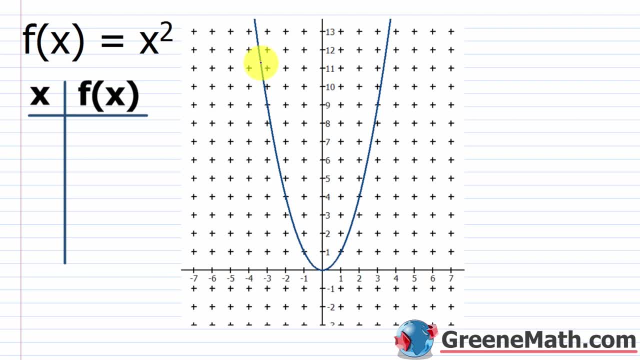 We can go through and get some points going, just so it kind of feels like we're completing the full process. So if we had f of x equals x squared and we wanted to sketch the graph, we'd get some points going. So let's just start with x equaling negative 2.. 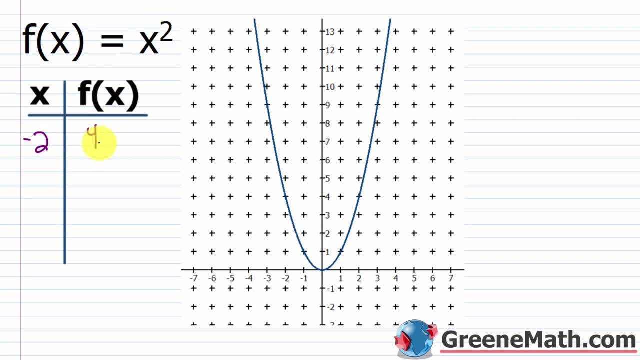 So if I plugged in a negative 2 for x, I would square it, I would get positive 4. Then let's do x equals- I don't know- negative 1. Plug in a negative 1 for x, square it, I get 1.. 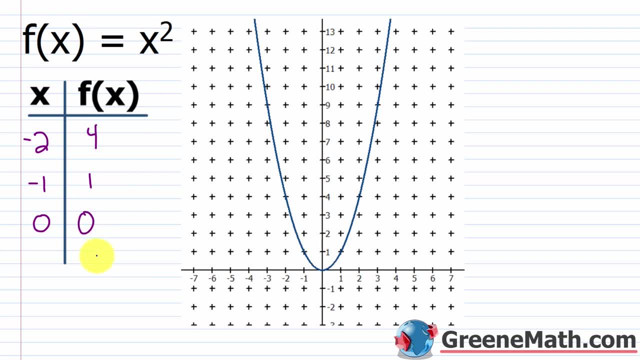 Then let's do x equals 0, square 0,, you get 0.. Then let's do x equals 1, square 1,, you get 1.. And then, lastly, let's get x equals 2, square 2, and you get 4.. 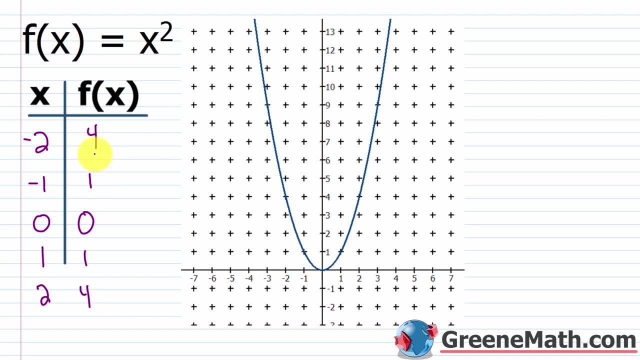 So we could plot these points: So negative: 2 comma 4.. So negative 2 comma 4.. Negative 2 comma 4.. That's right there. Then negative 1, 1.. So negative 1, 1.. 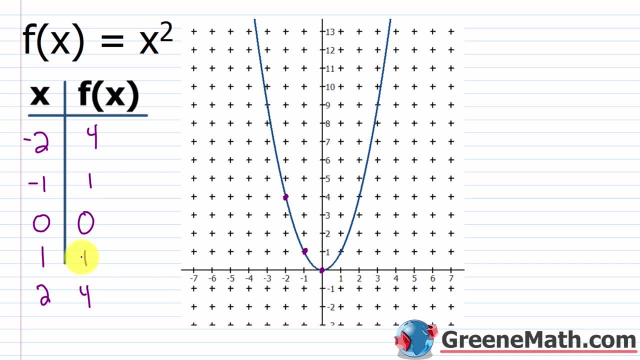 Then 0, 0.. So 0, 0, or the origin. Then 1 comma 1.. So 1 comma 1.. And then 2 comma 4.. So 2 comma 4.. You can see where we plotted our points. 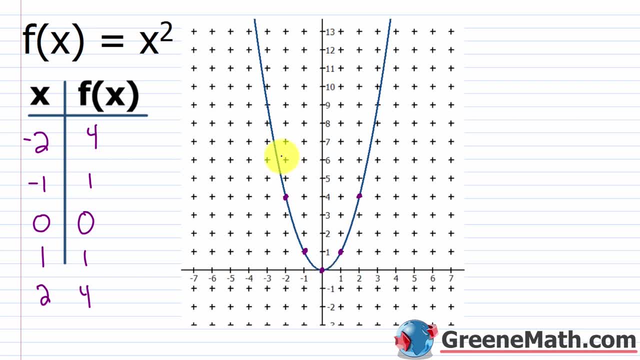 And again, if you were sketching this freehand, you'd have to get a lot of points kind of going this way to really get this thing accurate. So as you move forward, you really want to start relying on graphing calculators and graphing software. 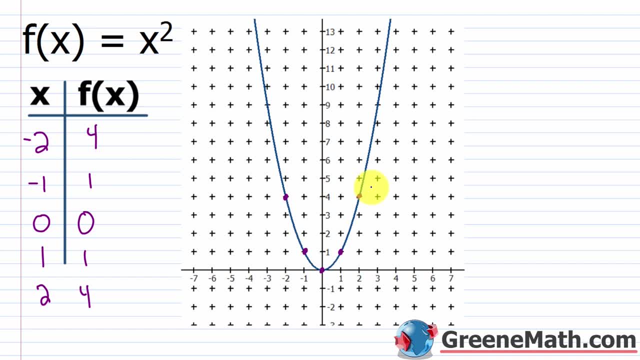 I realize that in some classes they're going to make you sketch some graphs. It's OK. Your teacher is going to understand that it's not going to be 100% accurate, OK. so now that we have the general idea of what a parabola is. 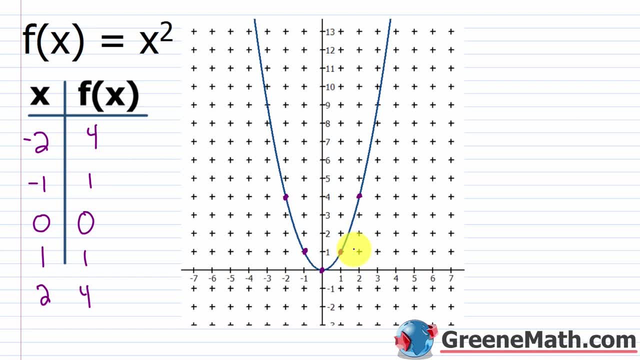 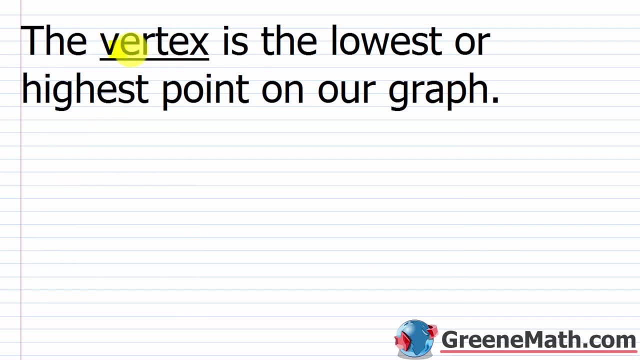 let's talk about a few important things. So the first vocabulary word that you're going to encounter is that of a vertex. So the vertex- and let me highlight that- is the lowest or highest point on our graph. So if we have a parabola that opens up, like in the example we saw, the vertex is the lowest. 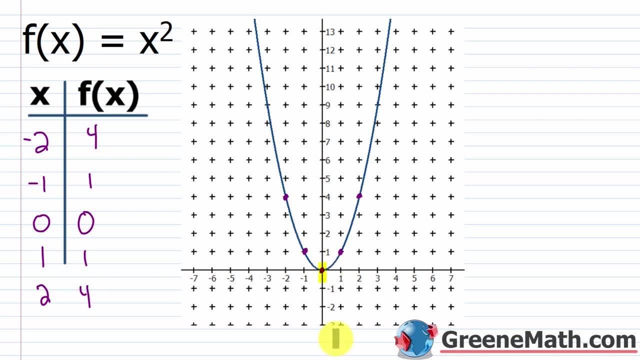 point on the graph. So in this case it's here. If we have a parabola that opens down, which we'll see at the end of the lesson, it's going to be the highest point on the graph. So one other quick point I want to make about parabolas. 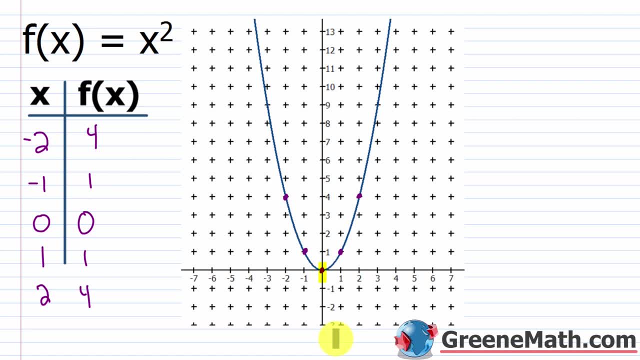 A parabola is symmetric about its axis. This just means we could fold our graph and the two curves would coincide. So you can imagine taking this graph- OK, This y-axis here- and just drawing a line down there. I know that's not perfectly straight. 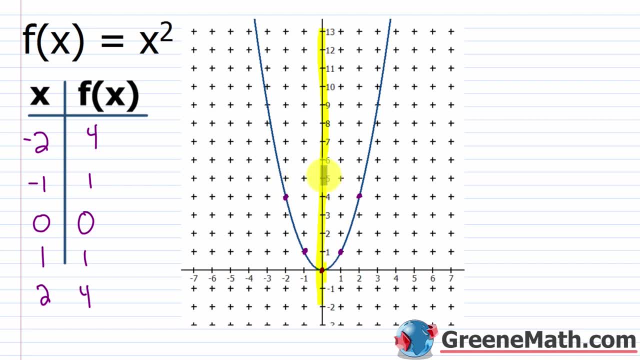 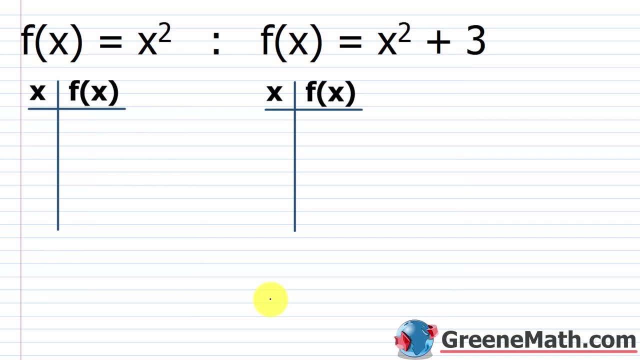 If you folded the two curves, you could see that they would coincide. So that's what they're talking about there. So now let's talk about shifts. This is the first thing you're going to come to when you start talking about parabolas. 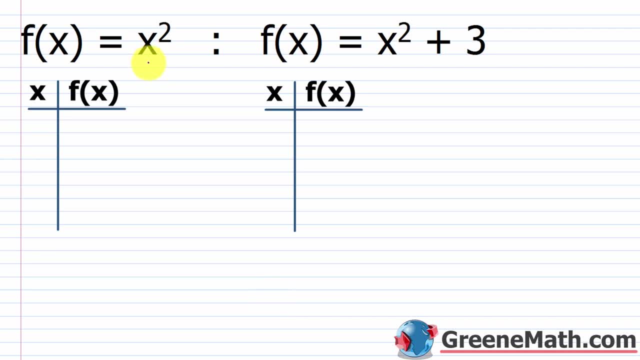 So we've seen the graph of f of x equals x squared. So the question is going to be: how can we use this to graph something like f of x equals x squared plus 3?? Well, without looking at the graph, let's just do some points for each one. 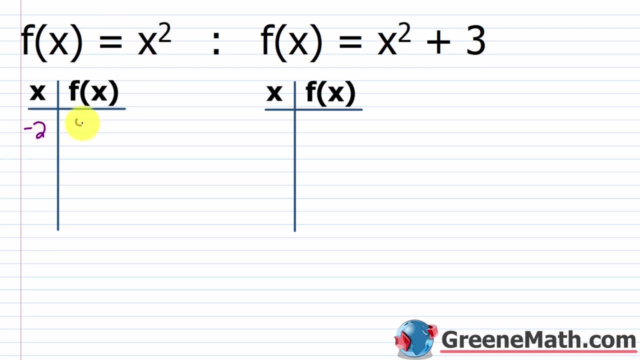 So we saw the points for this: when we know it's negative 2 and then 4, negative 1 and then 1, 0 and then 0,, 1 and then 1, and then 2 and then 4.. 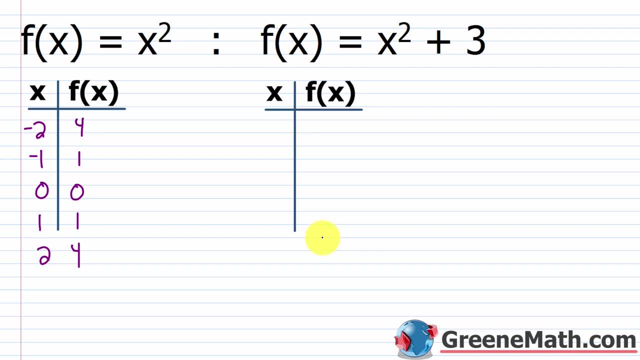 So let's use the same x values and see what we get for f of x or y values. If I had a negative 2 plugged in for x, what would be the result for y or f of x? Well, it's going to be the same thing as here. 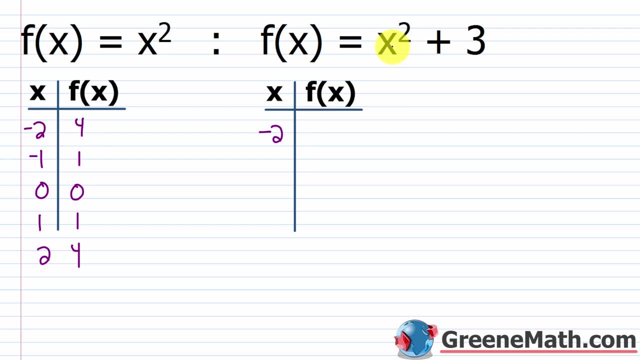 It's just going to be the same thing as here. It's just going to be the same thing as here. It's just going to be 3 units higher. right, because I'm taking this and then I'm just adding 3.. 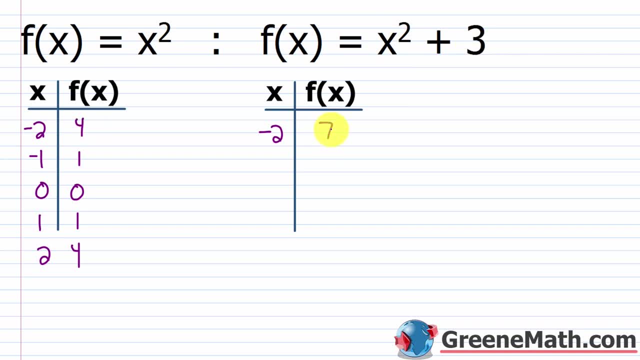 So I can just take this right here, 4, and say 4 plus 3 would give me 7, or I could manually do it: Negative 2 squared is 4.. 4 plus 3 again is 7.. So I can just take all these values and I could just add 3 to the y or f of x values. 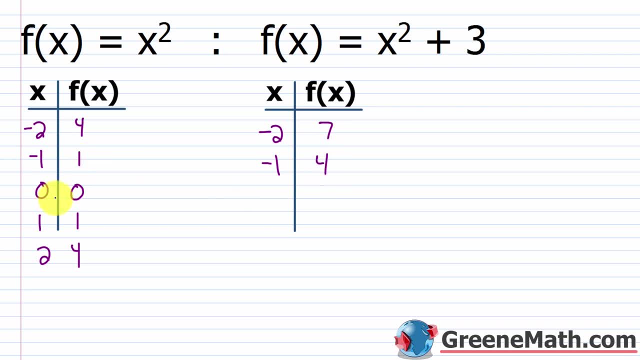 So negative. 1 would correspond to a y value of 4,, 0 would correspond to a y value of 3,, 1 would correspond to a y value of 3.. 1 would correspond to a y value of 4, and then 2 would correspond to a y value of 7.. 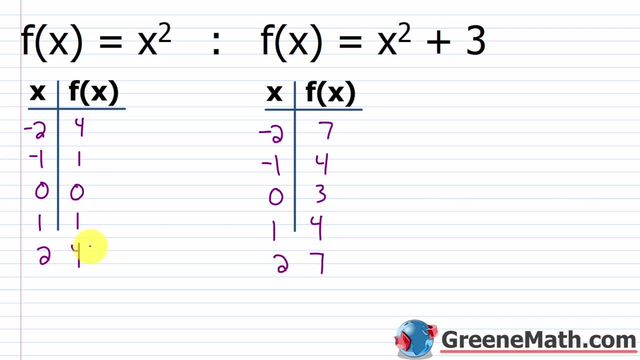 Again, all I'm doing is I'm taking the result from here and I'm just adding that 3 to it. Now, what do you think that does in terms of the graph? Well, for the same x value, okay, for the same x value. my y value, in every case, has. 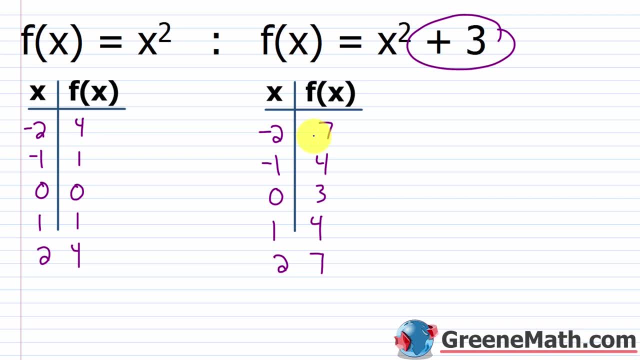 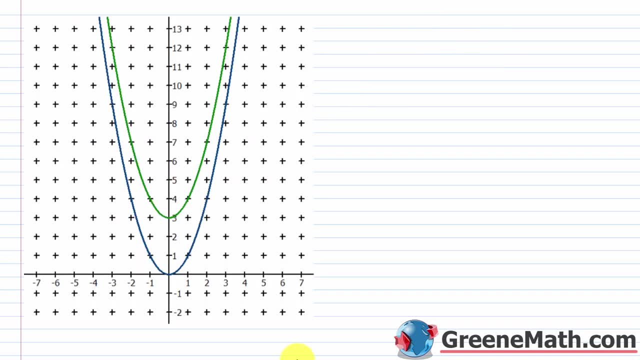 been increased by 3.. So that's going to create a vertical shift up by 3 units And you can see that the y value has been increased by 3.. And you can see this graphically. So this is the original. This guy right here is: f of x is equal to x squared. 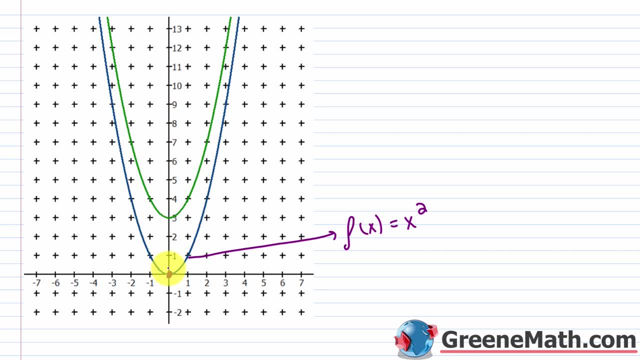 We see the vertex occurs at 0, 0.. We saw this, We talked about it already. This guy right here is the graph of f of x is equal to x squared plus 3.. The vertex, or the lowest point, occurs here at 0, 3.. 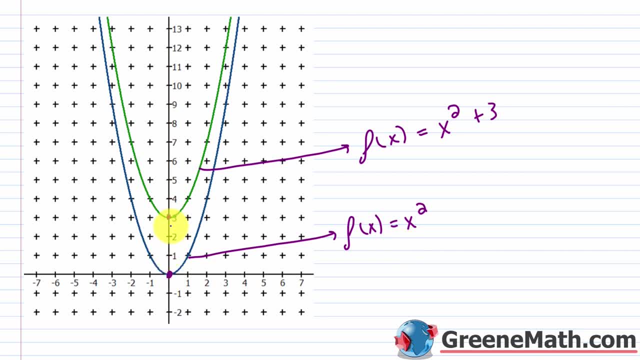 Everything has just been shifted up by 3 units, So the vertex went up 3 units. If you took a point like 1, 1, which is right here, if that shifted up 3 units, then that now occurs at 1, 4.. 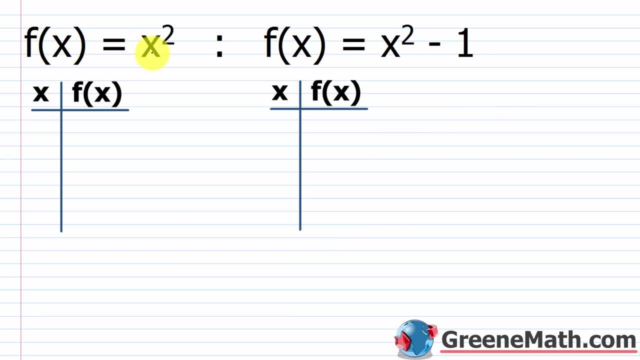 Let's take a look at another example. So again you have this f of x equals x squared. Now we're going to look at f of x equals x, squared minus 1.. Some of you can already guess that this will be a vertical shift down of 1 unit, right? 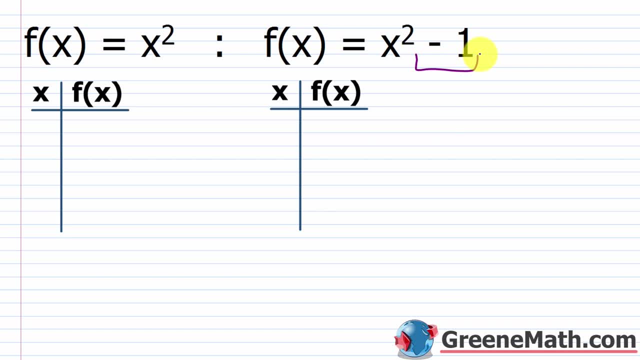 Because you have this minus 1. So the y values will just be decreased by 1 unit. So in other words, if I go through here and say negative 2,, negative 1,, 0,, 1, and 2.. 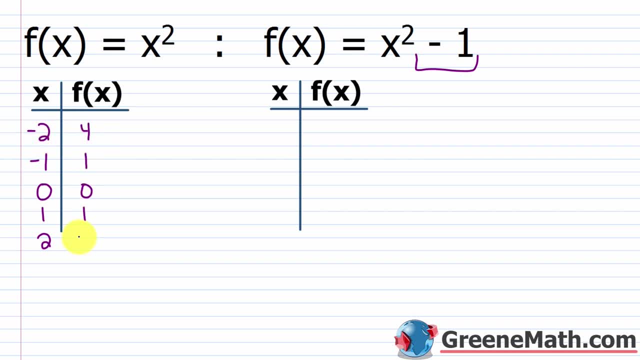 We remember, this is 4.. This is 1,, 0,, 1, and 4.. I can copy this. so negative 2, negative 1,, 0,, 1, and 2.. All I'm going to do is take these y values and I'm going to decrease them by 1, because 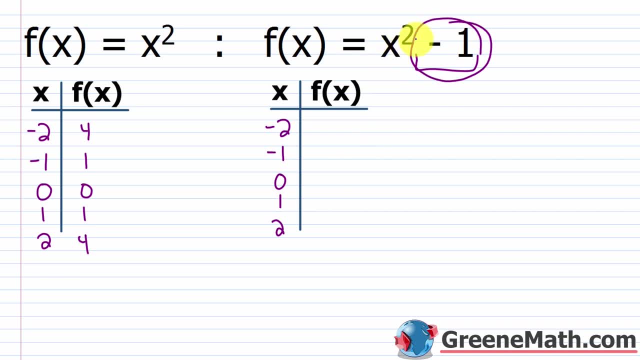 I'm plugging it into the same thing. The only difference is that minus 1 at the end. So I plug in a negative 2, I square it, I get 4.. I take away 1, I get 3.. 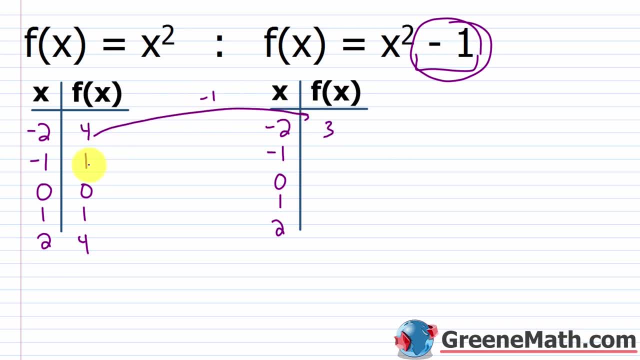 So this is 1 less, so minus 1.. This right here wouldn't be 1,, it would be 0.. 1 less This 0 would be negative 1, this 1 would be 0, and this 4 would be 3.. 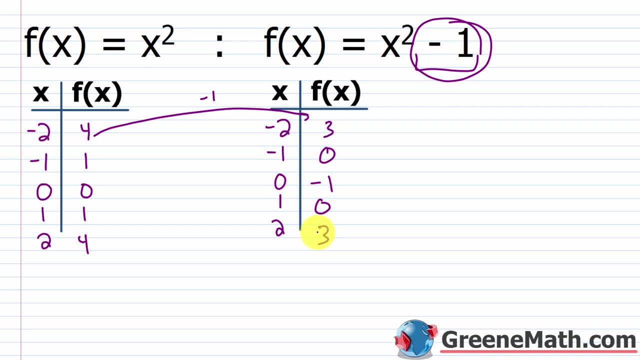 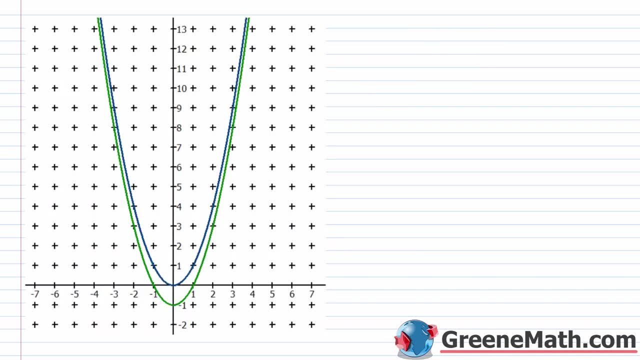 So for the same x value, the y value is 1 less. So this is a vertical shift of 1.. And you can see that here. So again, this is the original. This is: f of x is equal to x squared. and then this guy right here is your f of x is. 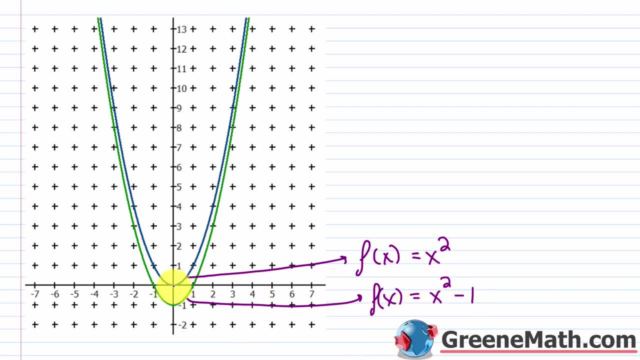 equal to x squared minus 1.. It's a vertical shift down. Here's your vertex: at the origin: 0, 0.. On the next equation, where we have f of x equals x squared minus 1,, the vertex moves down 1 unit. 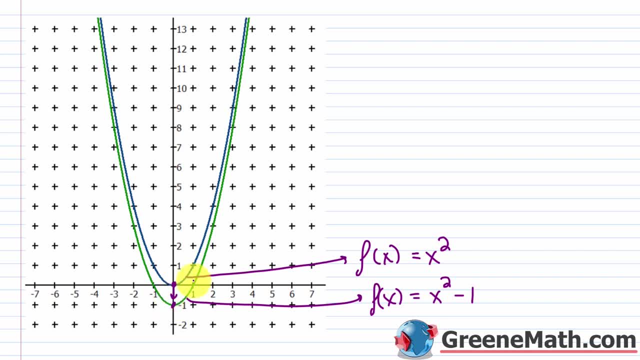 So it's at 0, 0.. Again, if I pick a point like 1, 1, which occurs on the original f of x, equals x squared. if I have an x value of 1 here in this equation it goes down by 1 unit for the y. 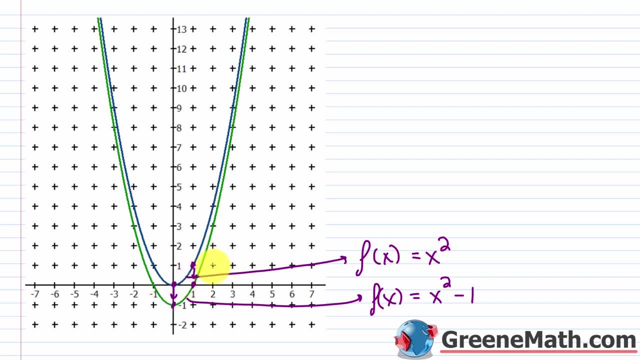 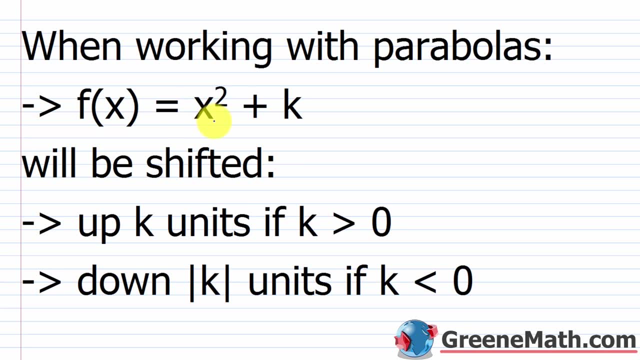 So that's going to be right here. So just shifted down by 1 unit. So pretty easy to understand that one. So, generically, when working with parabolas, if you have f of x equals x squared plus k, So plus k. 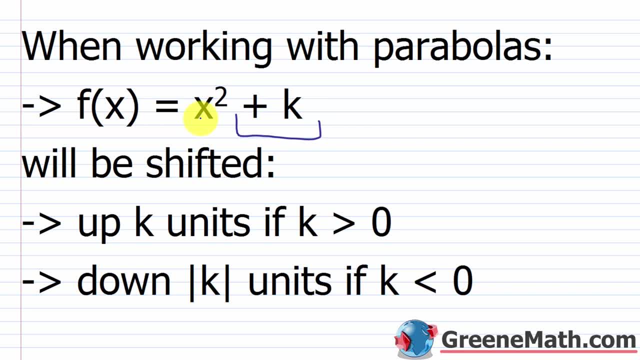 Okay, So what does f of x equals x squared looks like We're adding this k to it, So this will be shifted up k units if k is greater than 0.. So we saw that when we had f of x equals x squared plus 3, it was shifted up 3 units. 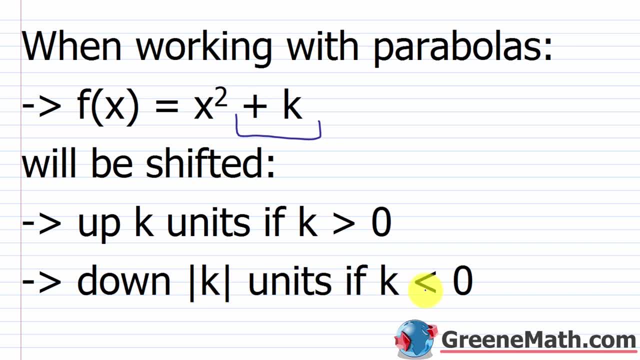 Then down the absolute value of k units if k is less than 0.. So when we had x squared minus 1, we think about that as plus negative 1.. We're really saying the absolute value of negative 1 is 1, so we're shifting it down. 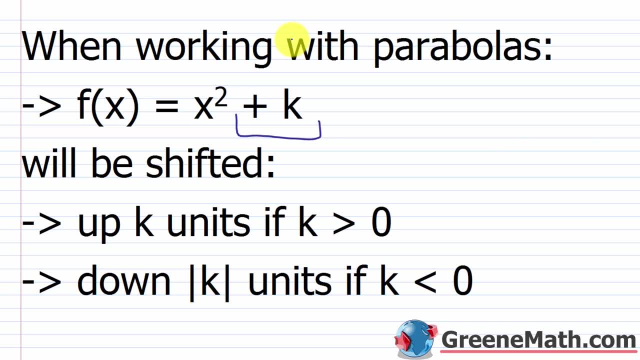 1 unit. We just saw that. So this is what you want to write down and kind of commit to memory. If you're working with f of x equals x squared plus k, your vertical shift will be up if k is greater than 0 or down if k is less than 0.. 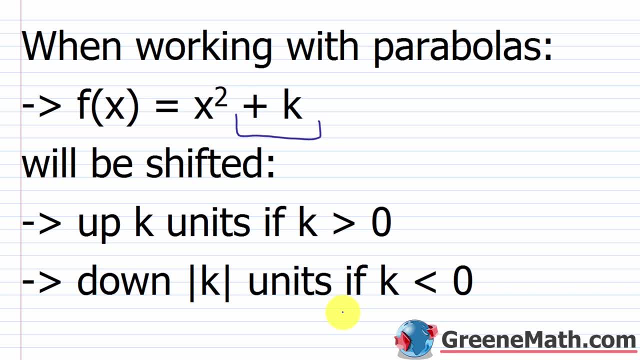 So if I had f of x equals x squared plus 10, I know that's a vertical shift of 10 units up. If I had f of x equals x squared minus 30, I know that's a vertical shift of 30 units. 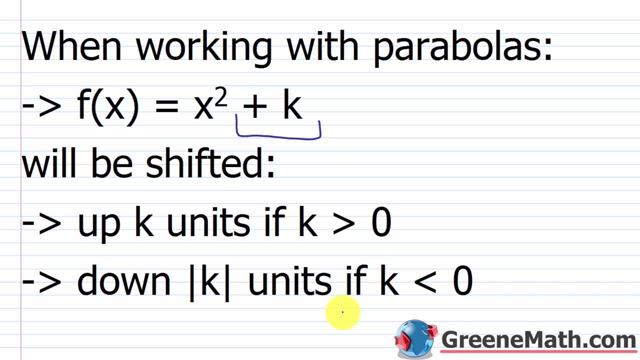 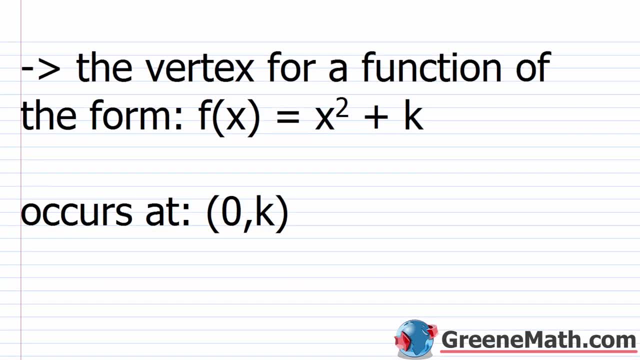 down Very, very easy. once you understand what's going on. That's a typical question. you'll get on a test. All right, so just some more kind of information. The vertex for a function of the form f of x equals x squared plus k is going to occur. 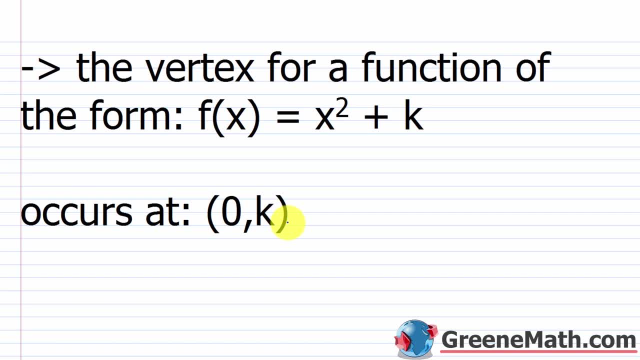 at 0 comma k. So you're thinking about the lowest point here. Well, if I plugged in a 0 for x, 0 squared would give me 0. I would be left with f of x, or you can think about that, as y is equal to k. 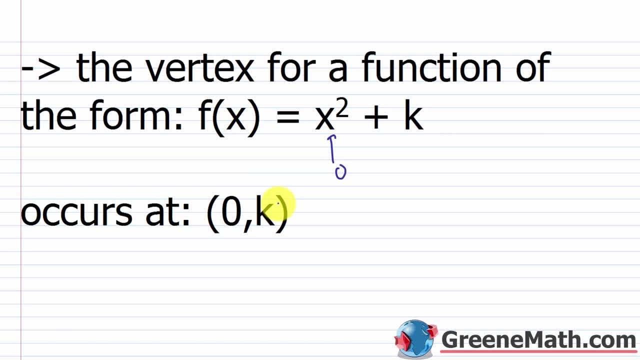 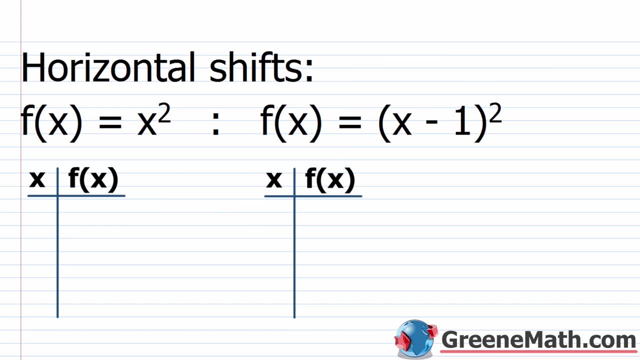 So 0 is the x location, k would be your y location or your f of x location. All right, so now that we talked about the easier scenario, which are vertical shifts, let's move on to horizontal shifts. Now, these might give you a little trouble mentally, but again it's like anything else. 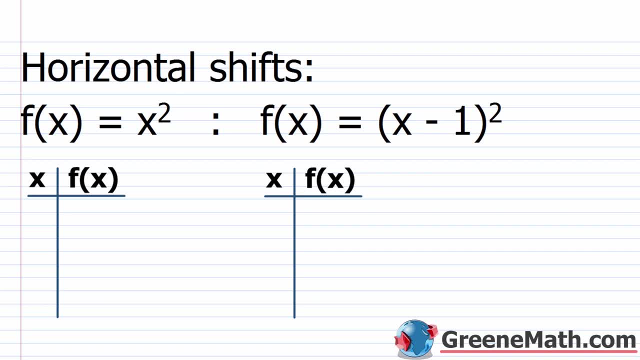 Once you kind of get used to it, it's really not that bad. So we have f of x equals x squared, and what we're going to compare this to? we have f of x equals x minus 1 squared. So let's just think about this. 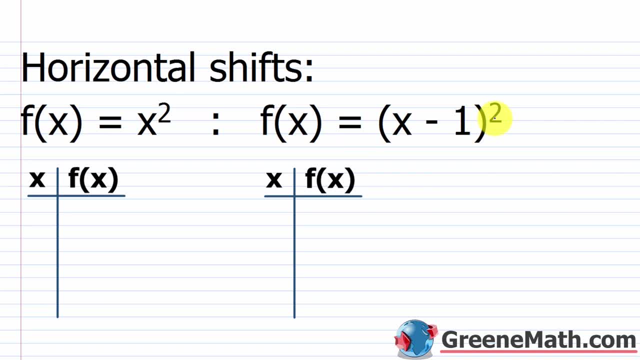 And again, this is something that really gives students a lot of trouble. Let's say I started with my typical negative 2, negative 2 squared, we know that's 4, and then negative 1, negative 1 squared is 1,. 0, 0 squared is 0, 1, 1 squared is 1, and 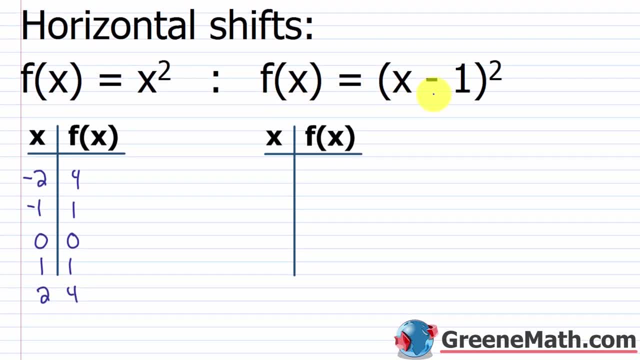 then 2, 2 squared is 4.. When we think about points for this guy right here, if I had a negative 2 plugged in for x, what would happen to y? Well, I plug in a negative 2.. Negative 2.. 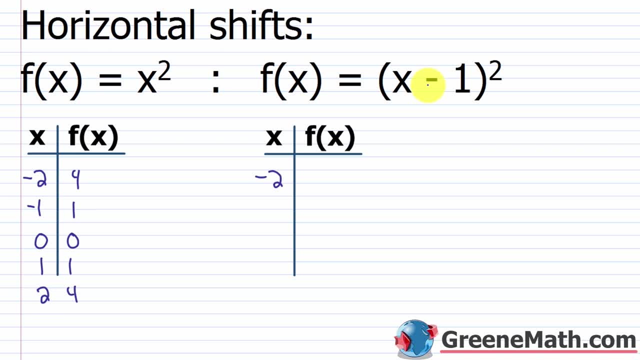 Negative 2 minus 1 would be negative 3. Negative 3: squared would be naught, Okay. so you say, well, I don't really see what happened, Okay, so let's keep going. So you plug in a negative 1.. 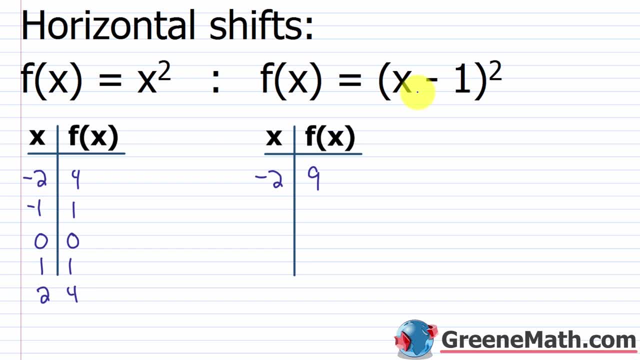 Negative 1 minus 1 would be negative 2.. Negative 2 squared would be 4.. So negative 1, and then you'd have 4.. If I plugged in a 0, 0 minus 1 would be negative 1, negative 1 squared would be 1.. 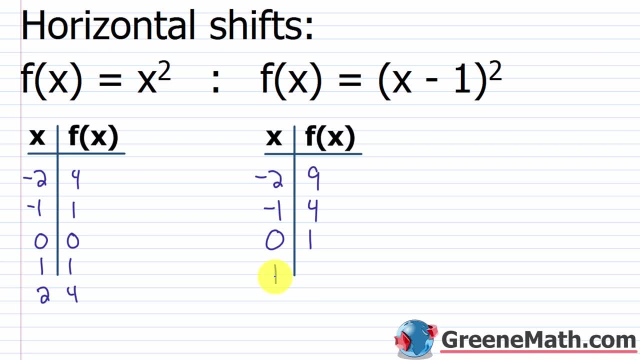 If I plugged in a 1, 1 minus 1 would be 0.. 0 squared is 0.. And then, if I plugged in a 2, 2 minus 1 would be 1, 1 squared is 1.. 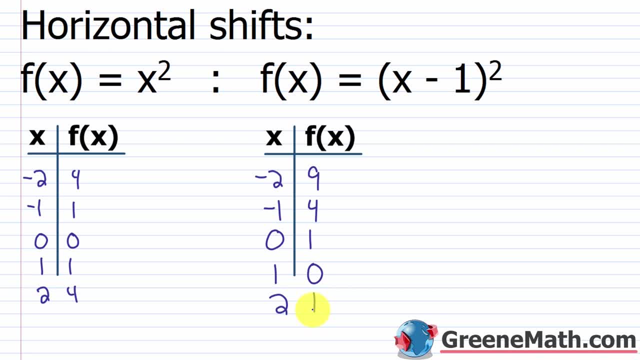 So what's going on here? Well, what's going on is that the x value must be 1 unit larger to obtain the same y value. This is going to create a horizontal shift to the right by 1 unit because, again, let's. 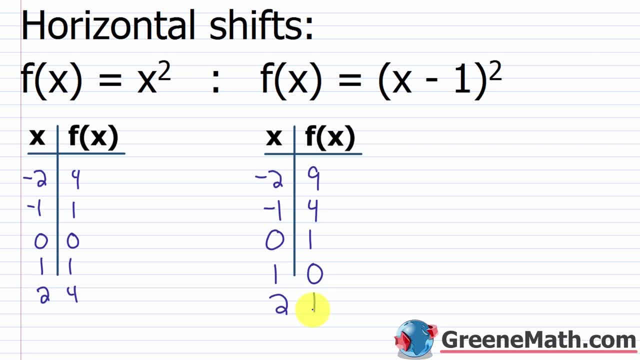 just think about this: The x value needs to move 1 unit to the right or be 1 unit larger to obtain the same y value. So, just when we take a look at the points, an x value of negative 2 corresponds to a. 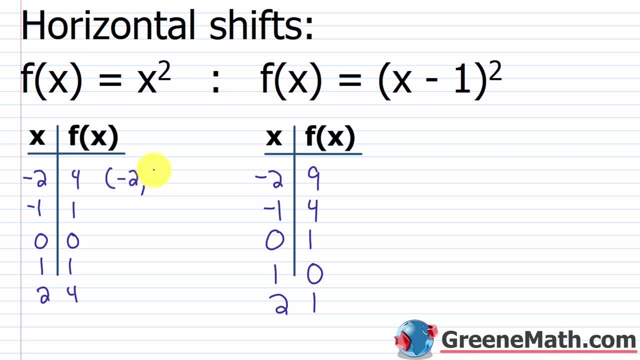 y value of 4.. An x value of negative 2 corresponds to a y value of 4.. Here I've got to increase the x value by 1 or go from negative 2 to negative 1 to get a y value of 4.. 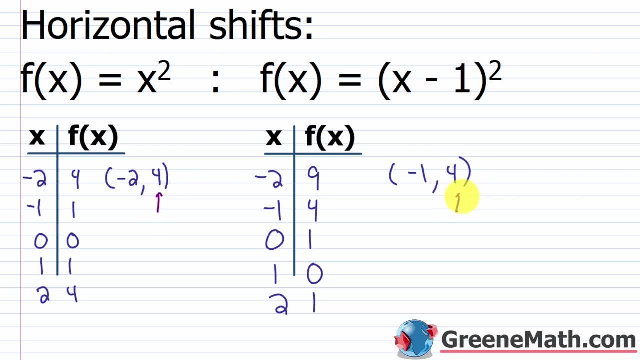 So I've got the same y value here and here, but my x value increased when I went to this guy by 1.. I went from negative 2 to negative 1.. So again, that's what's going to create this horizontal shift to the right by 1 unit. 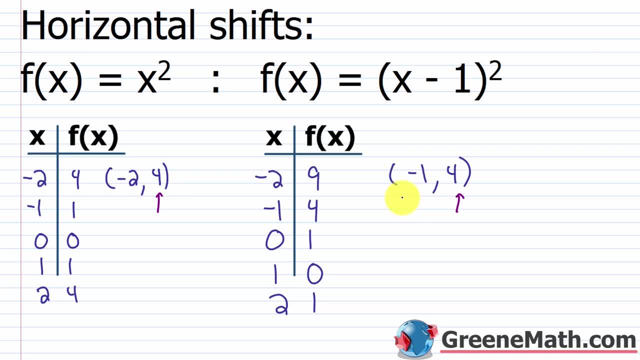 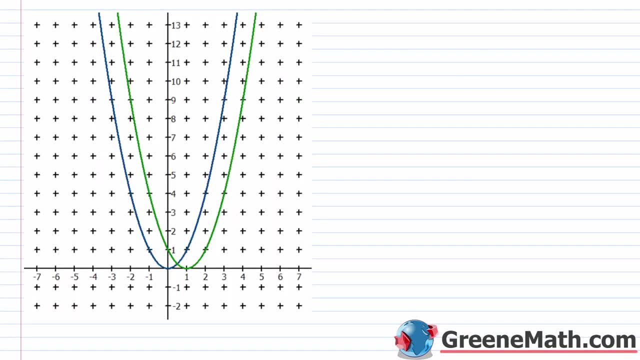 It's because to get the same y value or to be in the same vertical location, I've got to move to the right by 1 unit. So here you can see the two graphs On the same coordinate plane, this blue guy right here. that's our f of x equals x squared. 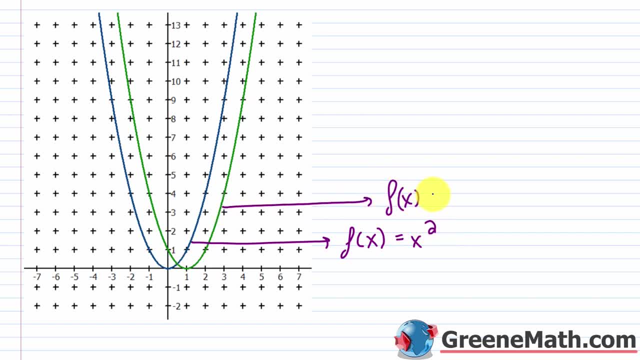 And this green guy right here. this is: f of x is equal to the quantity x minus 1 squared. And again, all this is is a horizontal shift to the right by 1 unit. For this guy, the vertex occurs at: So for this guy, I'm just going to shift to the right by 1 unit. 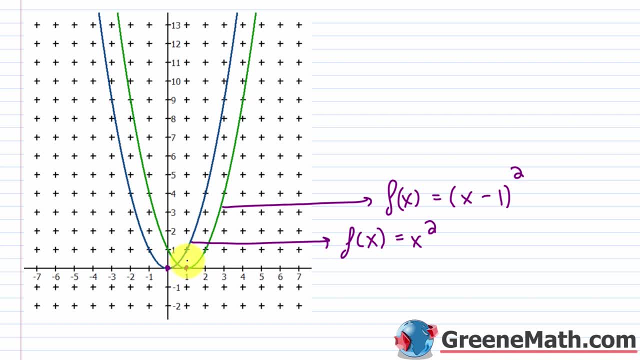 So the vertex occurs at: Okay, so everything is to the right by 1 unit. So again, if I look at a point like this: has moved 1 unit to the right. So now I'd have an x value of 2 with a y value of 1.. 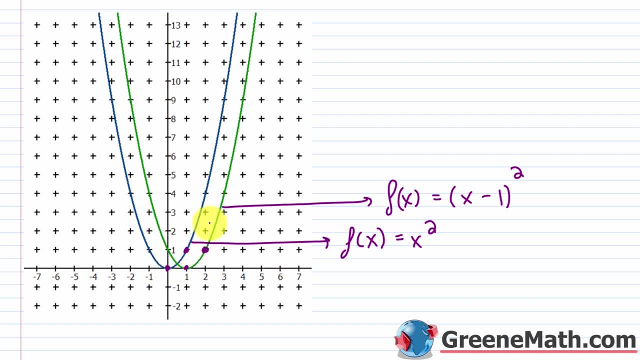 If I have an x value of 2, that corresponds to a y value of 4, for f of x equals x squared. For this guy I now need an x value of 3 to correspond with a y value of 4.. So again, I'm just shifting everything to the right by 1 unit. 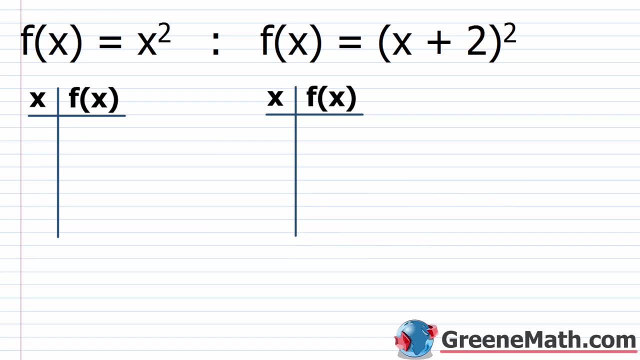 Now let's take a look at another example of this horizontal shift. So we have: f of x equals x squared. again, You're always going to see that- And we're comparing this to f of x equals the quantity x plus 2 squared. 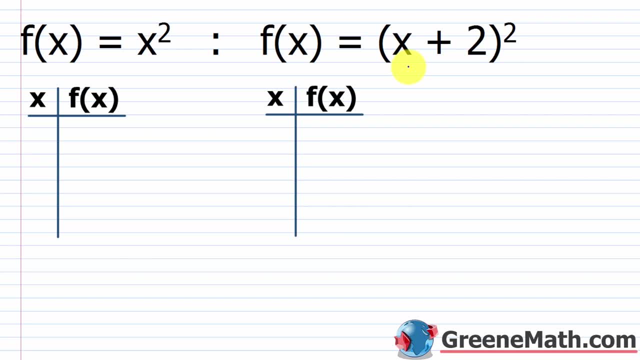 So now we're adding 2 to x. So think about this. This is going to go in the opposite direction. now, The way you want to think about it is that the x value must now be 2 units smaller To obtain the same y value. 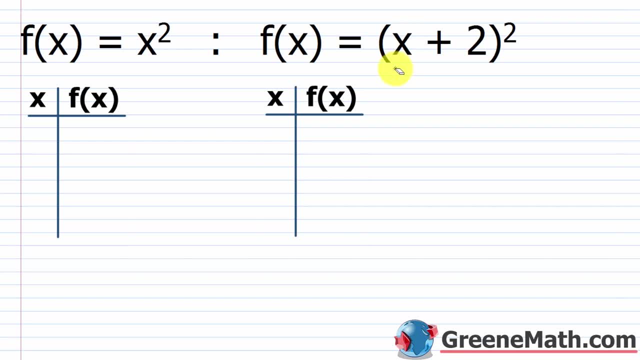 Okay, 2 units smaller And we can just do some points to see that. So again, we go with our. You probably memorized this by now. This is going to be 4.. This is going to be 1,, 0,, 1, and 4.. 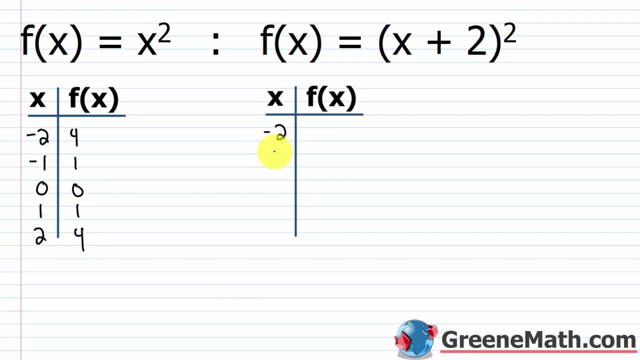 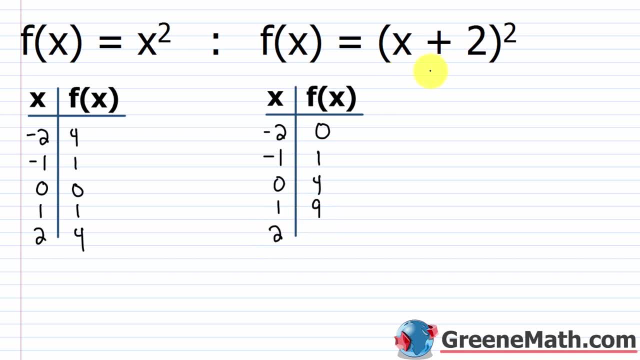 And then we just thirteen double zero. So minus n can be 2.. Always take theyg番 in two: Plus, I'm going to subtract over the n in n, And then minus n, I'm going to subtract in 4. So less than minus n. 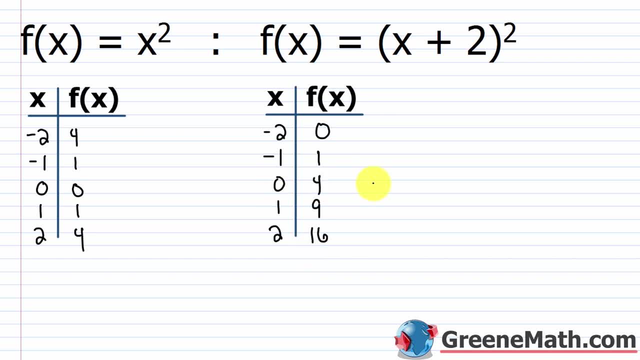 So less than n, I'm going to subtract 5.. So minus th increase in n, I'm going to subtract over the n And minus 2 over 0.. So with our y comes to 0.. You get 6.. But I'm going to subtract over the n. 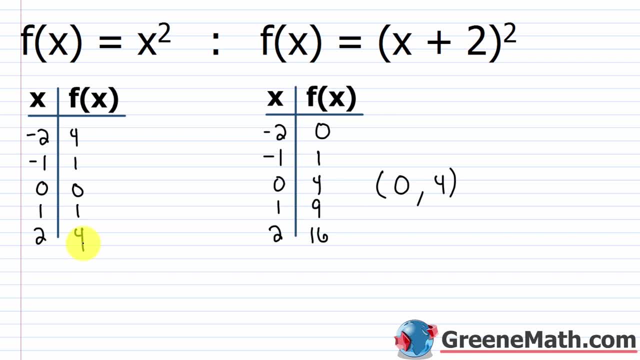 And then plus n takes 2.. So plus n in over 0. Plus 1.. So 1 in x equals 1 over 0. I'm thinking about an x value of 2. So 2, 4.. So in other words, this guy right here, this 0, is 2 units less than this 2 here. 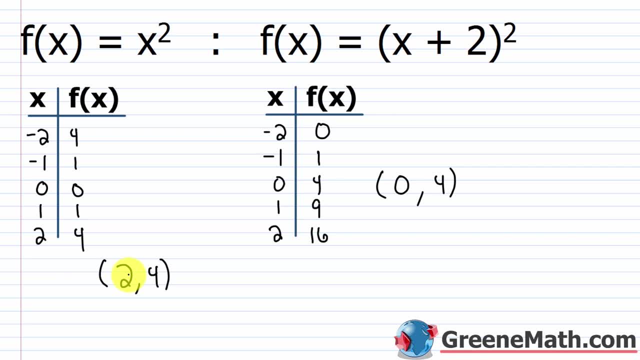 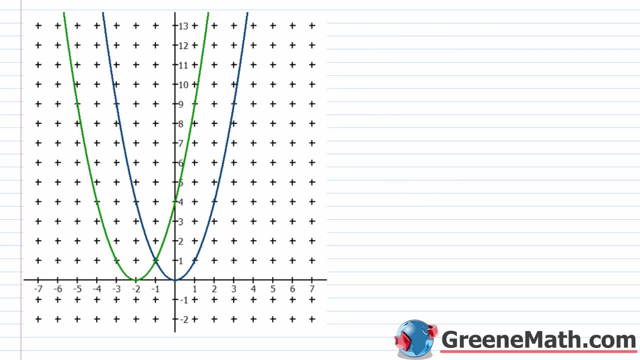 Two units less in terms of x. we're moving two units to the left on the x-axis to get to that same y value of 4.. And you can see it when you look at the graph. So here's your vertex. here, for again, f of x equals x squared. and then here's your. 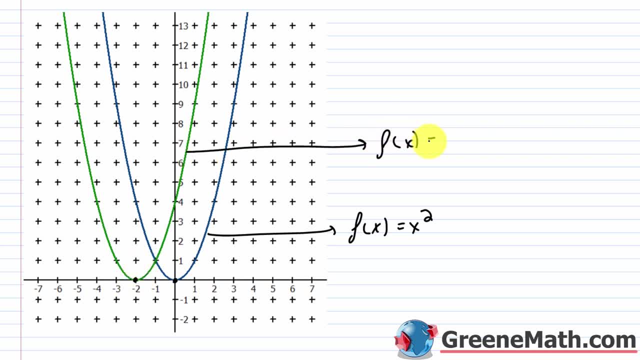 vertex for f of x is equal to the quantity x plus 2 squared. You can see everything has just shifted two units to the left. Here it's at 0, 0.. Here it's at negative 2, 0.. So my x location just went two units to the left, or decreased by 2.. 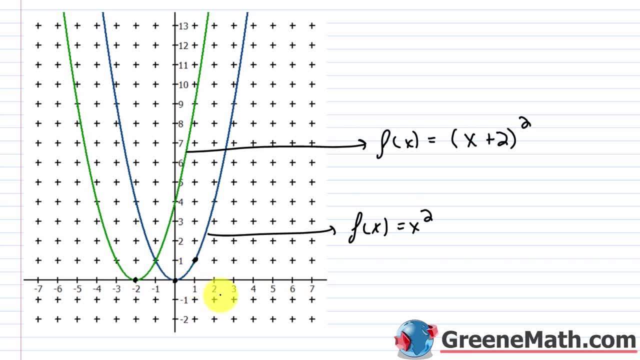 You can think about this point 1, 1 that we keep going to. Well, if I decrease my x value by 2, so I go 1, 2 units to the left, I know that I'm going to have my y value of 1.. 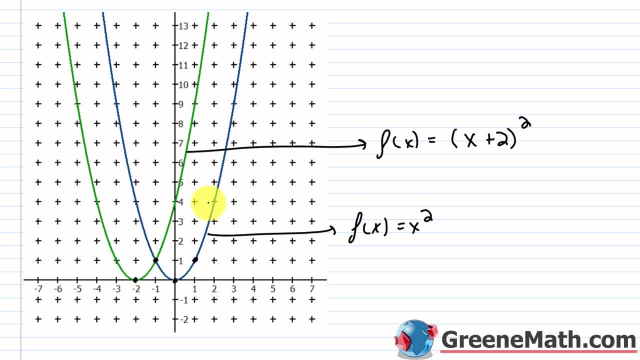 You can see that there. If I take a point like 2, 4, that's here, If I decrease my x value by 2 and I go from 2 to 0, I'm going to see 0, 4.. 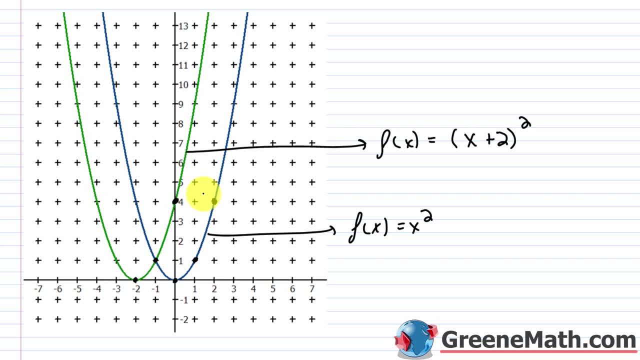 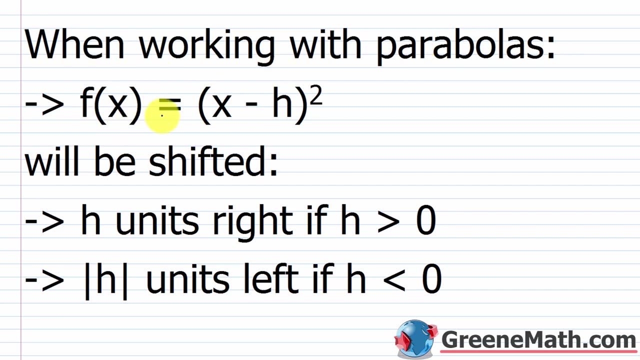 So the same y location occurs when the x value is 2 units left or 2 units less. So this is what's creating the horizontal shift, All right? So here's the kind of cheat sheet for this When working with parabolas. again, if you see, f of x is equal to the quantity x minus. 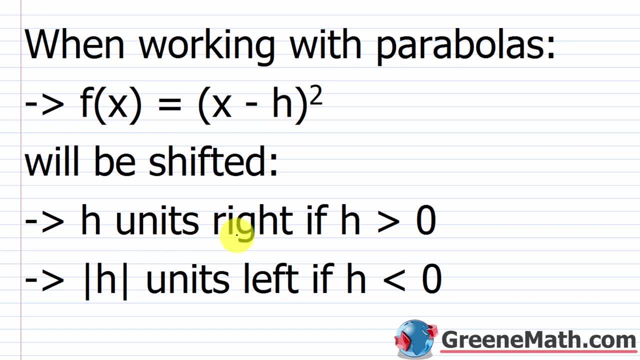 h and this is squared. this will be shifted h units to the right if h is greater than 0.. Okay, H units to the right. So if it's x minus 1, then it's going to shift one unit to the right. 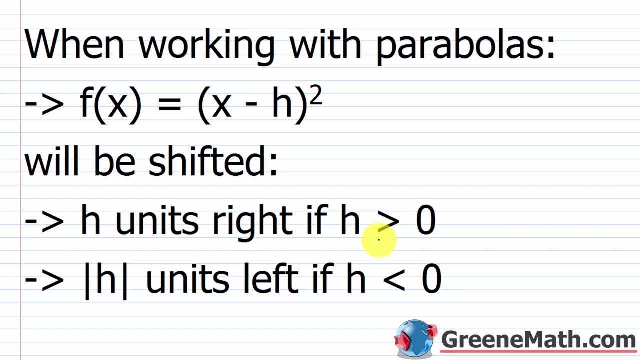 Because, again, the x value needs to be one unit larger to obtain the same y values, and that's what creates that shift. In the other scenario we say the absolute value of h units left if h is less than 0. So this gets a little bit tricky. 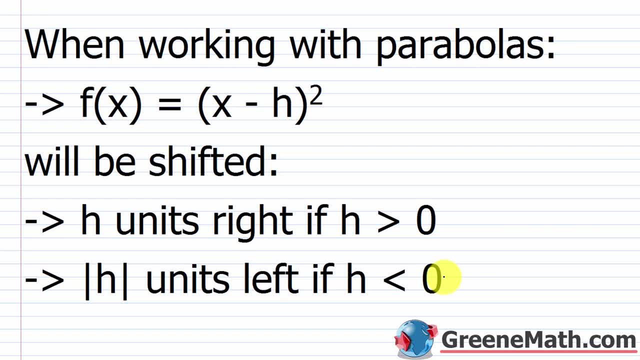 You're thinking about things like, let's say, you saw the quantity x plus 3 in there. Well, really I could write this as: f of x is equal to the quantity x minus a negative 3.. Right, Because we're always keeping that minus symbol in there. 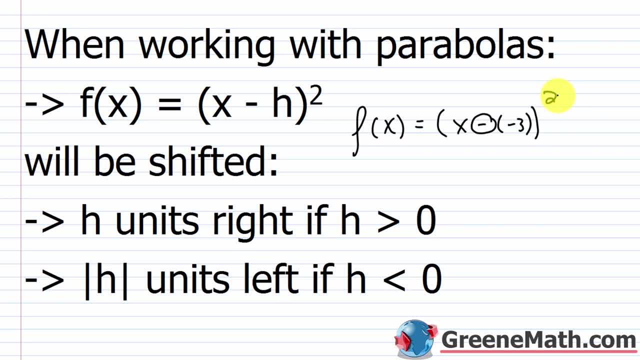 So this is squared. But if you see plus 3, you know that you're just going to move it. You're just going to move left by 3 units. Okay, You don't need to go through all this. Really, what this is technically saying is that you take the negative 3, you take the. 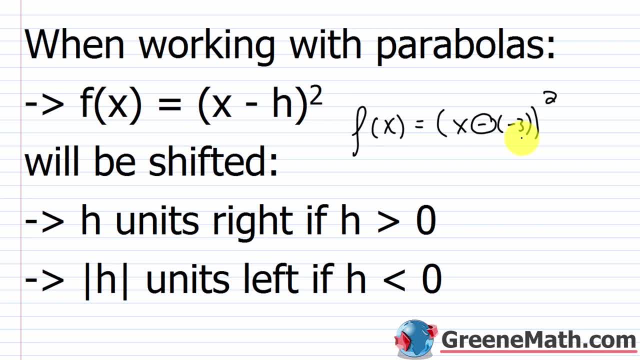 absolute value of that, you get 3.. You're going to move 3 units left, But again, this is ultra complicated. When you see a minus sign and a positive number behind it, you know you're moving right by that number of units. 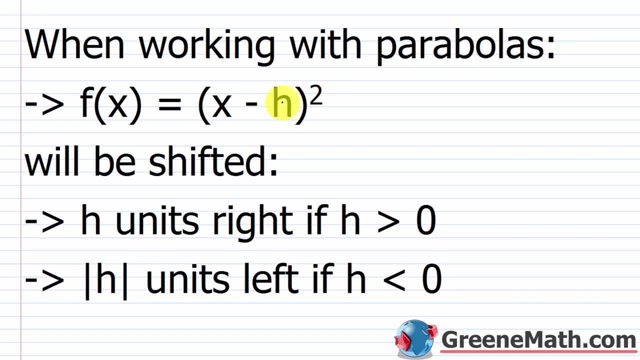 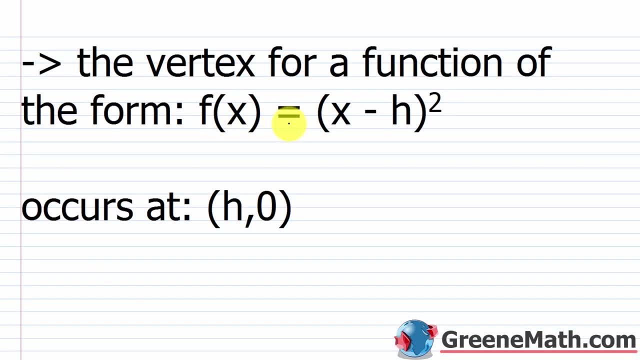 When you see a plus sign and a positive number, so like x plus 3,, for example, you know you're going to move left by 3 units. Okay, So the vertex for a function of this form, if we have f of x, equals the quantity x minus. 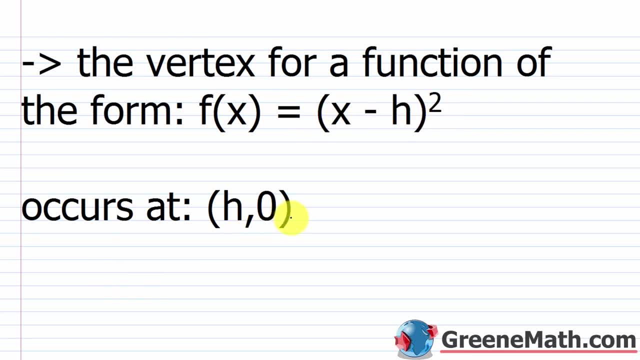 h squared, this is going to occur at h comma 0. So in other words, if I plug in an h here for x, that's going to be h minus h, which is 0, 0 squared is 0. So that's giving me the lowest point for y or for f of x. so the lowest point for the. 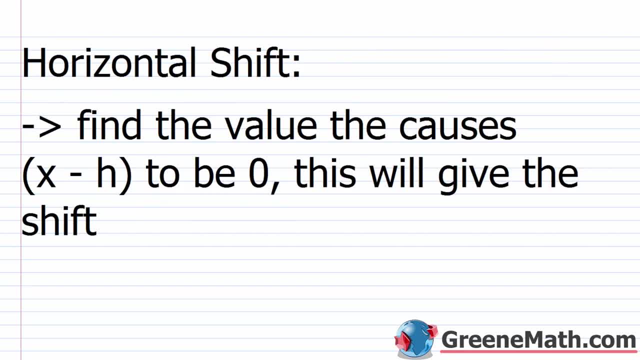 function All right. So if you're on a test and you're really, really confused, you don't know what's going on. horizontal shifts give students the most trouble. You can kind of go through it With the vertical shifts. they really get it right away. but a lot of students with 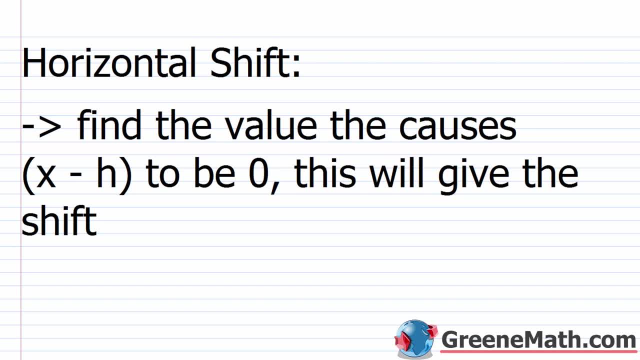 the horizontal shifts are just like. I don't know what's going on. I can't figure this out. Just find the value that causes x minus h to be 0. This will give you the shift. So if it's- let's say I had f of x- is equal to the quantity x minus 30 squared. 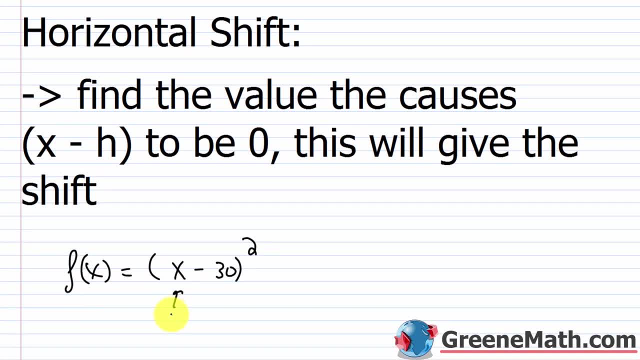 What would make this equal to 0?? Well, if I just plugged in a 30 for x, 30 minus 30 would give me 0.. Okay, 0 squared would be 0.. So if I'm plugging in a positive 30, you think about positive as moving, right, right? 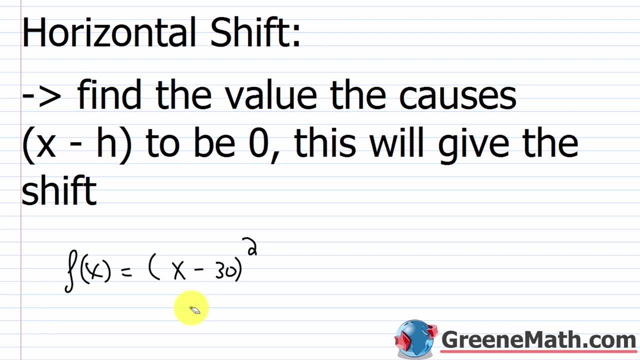 So I'm moving right: 30 units. So it's a 30 unit to the right shift, horizontal shift to the right: 30 units. however, you want to think about that. If I replace this with 25, we know the shifts would be 25 units to the right, because I'd 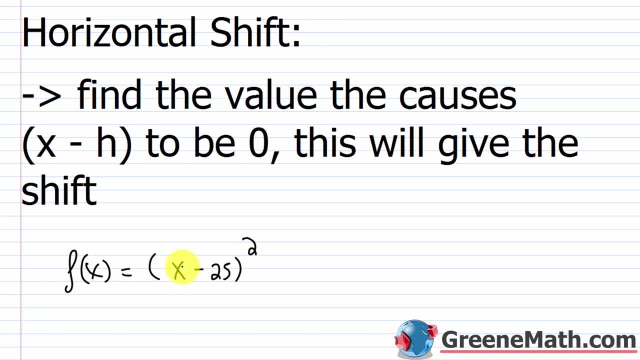 plug in a 25 in for x and I would get a 0 there. If I change this to a positive, let's say a positive 7.. How could I make this 0?? We'll plug in a negative 7 for x. 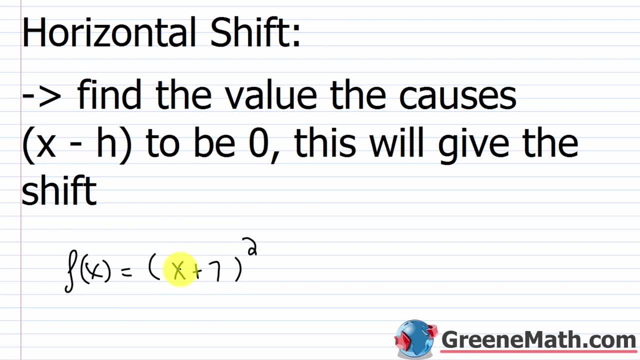 Negative. 7 plus 7 is 0. So you think about negative as moving to the left, a negative direction. So I'm shifting to the left 7 units. So this is a little trick, It's not something to confuse you. 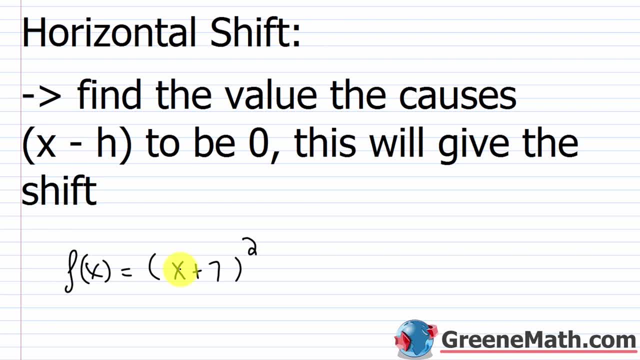 If you're lost when you're talking about horizontal shifts, just find the value that causes the quantity x minus h to be 0.. Okay, So forget about the square, Forget about the f of x, Forget about the notation. What would cause this to be 0?? 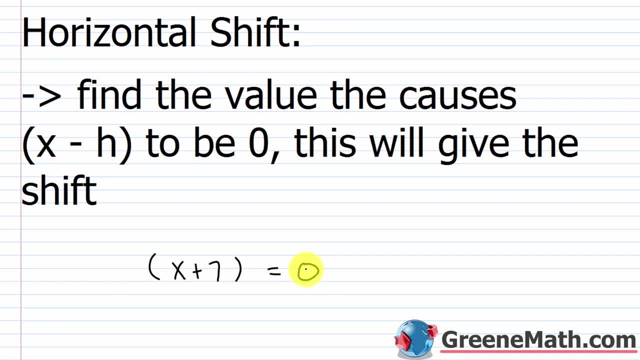 Give that answer and you found your shift. If it's negative, you're moving to the left. If it's positive, you're moving to the right. So here I'd need a negative 7 for x. So I'm moving to the left- 7 units. 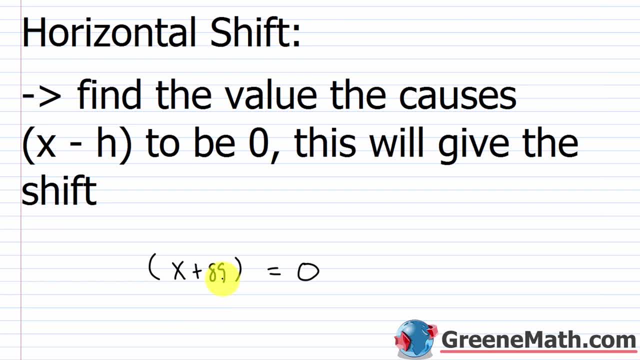 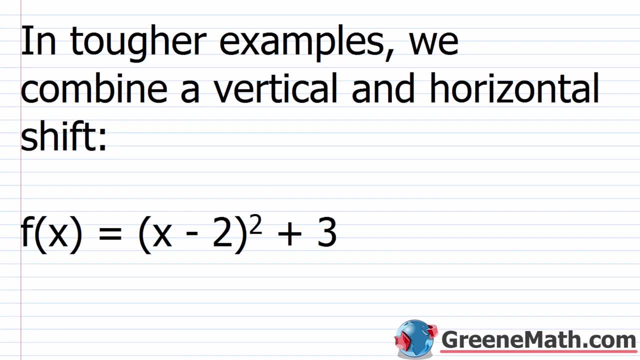 If this was plus 89, I would need to put a negative 89 in there. So I'm shifting 89 units to the left, right, So on and so forth. So in tougher examples we combine a vertical and horizontal shift. 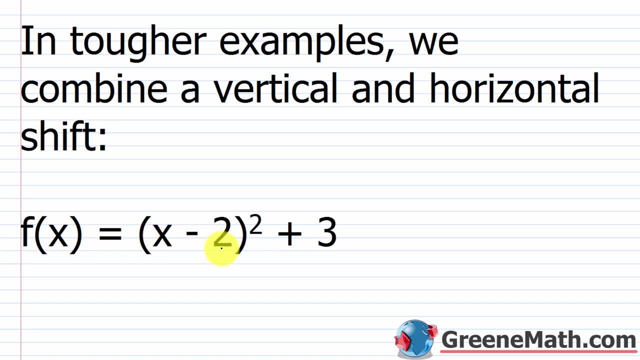 So you'll see these examples where you see f of x equals the quantity x minus 2, squared then plus 3.. So some of you get it right away. You just combine the two shifts. So if I think about the horizontal shift, I just look at this and I say, okay, I have. 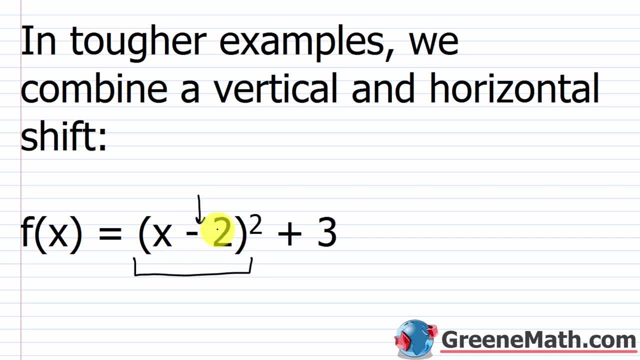 a negative 2, there a minus 2.. I know that corresponds to a shift to the right, So a shift to the right by 2 units. Then this plus 3, here is a shift up by 3 units, So a shift up. 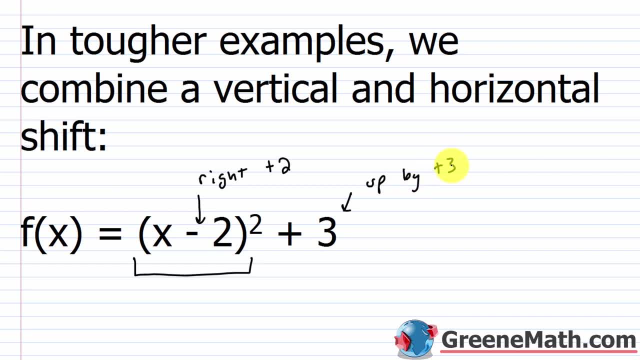 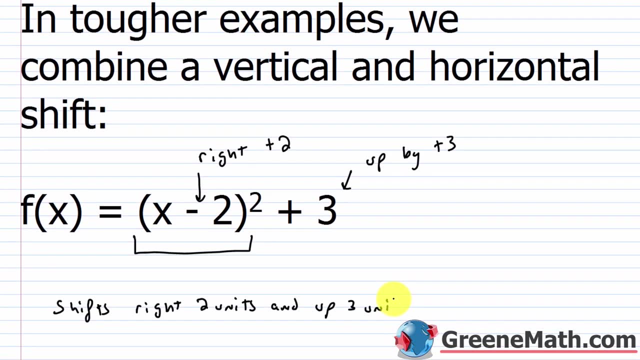 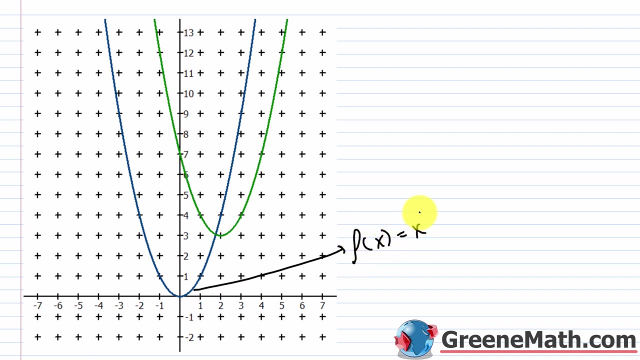 Up by 3 units. So this guy would shift. So it shifts right: 2 units and up 3 units. okay, Pretty easy overall. So you can see this graphically again. this is the original f of x equals x squared. 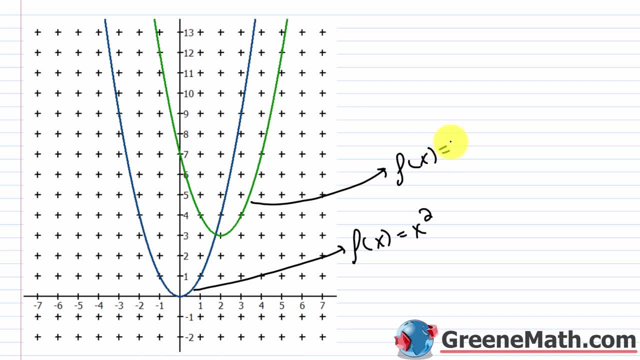 And then this guy right here is: f of x is equal to. We have the quantity x minus 2 squared, and then plus 3.. So here's your vertex, Here's your vertex. So that's what I look at, And you just think about the fact that, okay, it's a shift of 2 units to the right. 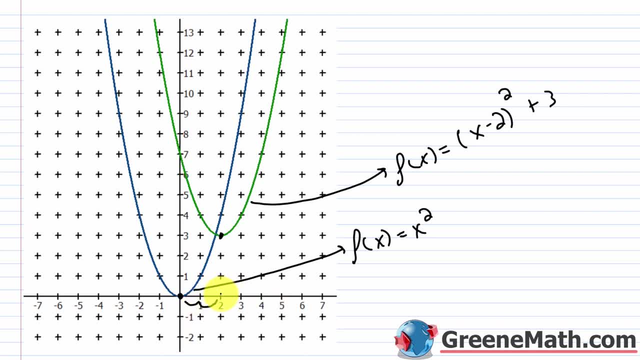 So I'd go 1,, 2 units to the right And then 3 units up. So 1,, 2,, 3 units up. So you go from there to there. So 2 units to the right, 3 units up. 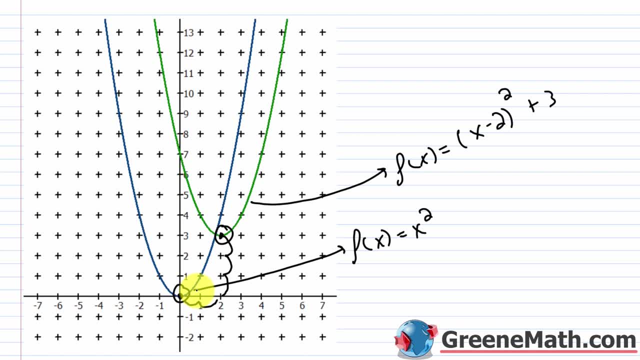 This is all you really need to do on your test, especially if it's presented to you in a graph. You can just count the shift to the right Or the shift to the left, And then count the shift up and down right. 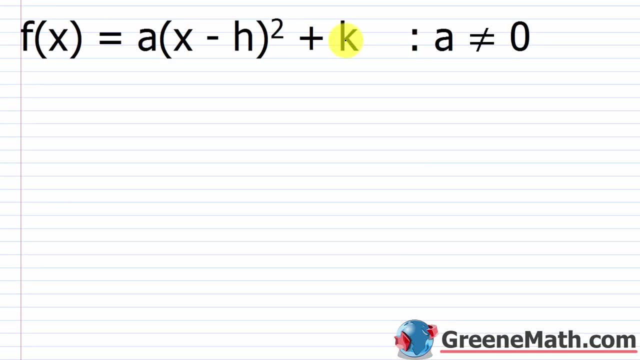 So very, very easy to do if you get it on a graph. So when we see the format f of x equals a times the quantity x minus h squared plus k. where again a does not equal 0, we can say the vertex occurs at h comma k. 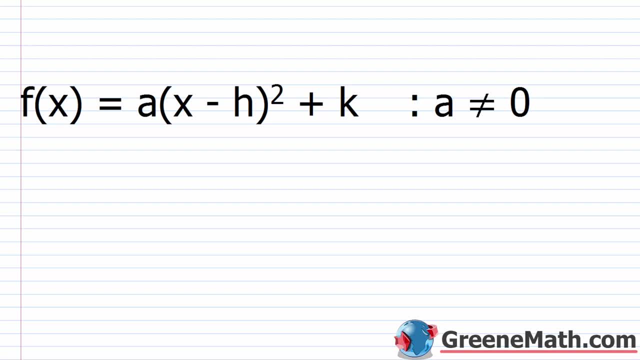 And why is that the case? Let's go back up. We're thinking about how to make this in this case, because this is positive as low as possible. So if I plugged in an h for x, h minus h would give me 0.. 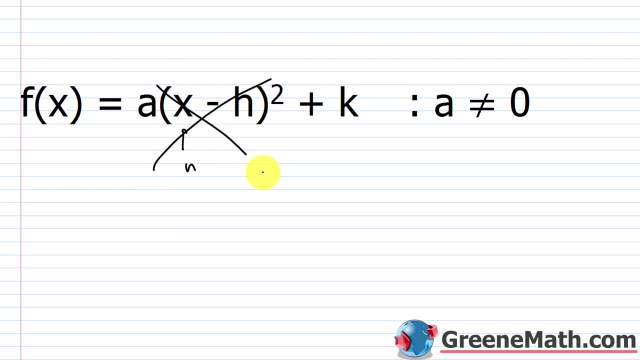 0 squared is 0.. 0 times a is 0.. So this is essentially gone. So I'm just left with k. All right, So that's the lowest it can be. Plug in an h for x. That eliminates that. 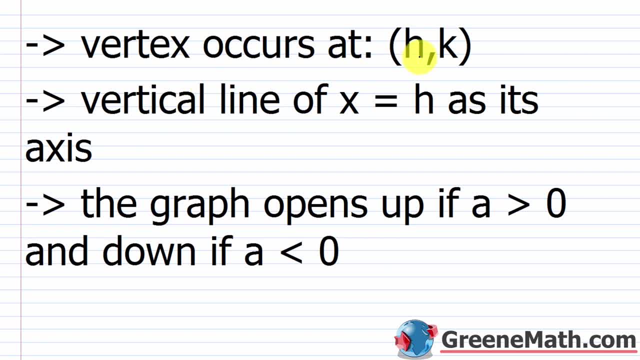 It wipes it out. I'm just left with k. So that's why our vertex occurs at h comma k. Then we have a vertical line of x equals h as its axis. Again, that's going to split it in half. If you fold on that, the two curves are going to coincide. 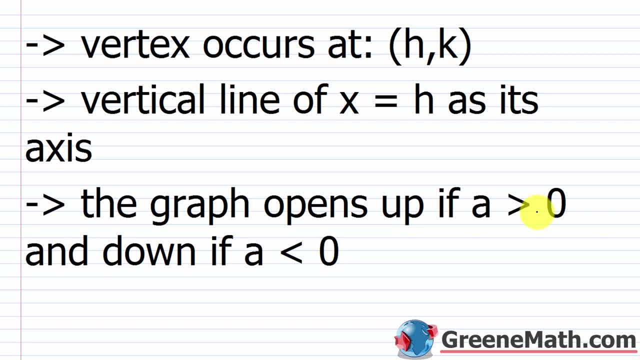 And then the graph opens up if a is greater than 0.. Right, So the coefficient of the squared variable is positive and it's going to open down if a is less than 0, or again, the coefficient of the squared variable is negative. 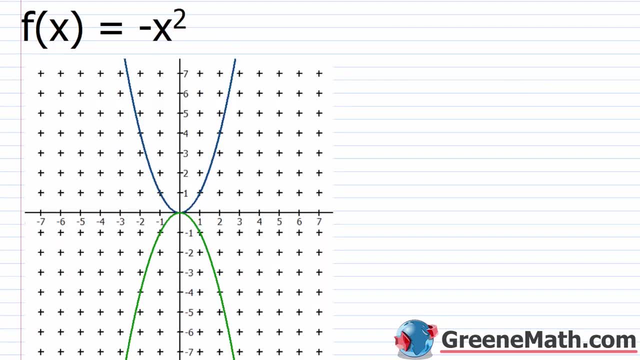 All right, So overall, not too difficult, just things you need to get used to. A lot of it is just memorizing what you need to do And then, as we move forward, we're going to start seeing some downward-facing parabolas. 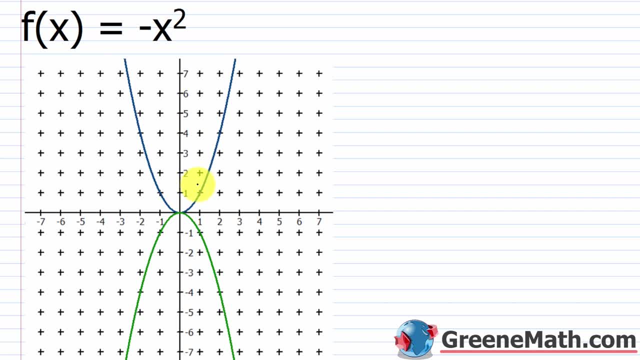 So all we've seen so far are the parabolas that open up. So the f of x equals x squared, that variety Now we're going to look at. f of x equals negative x squared. So the trick here is that if you have a negative coefficient on the squared variable, so you're. 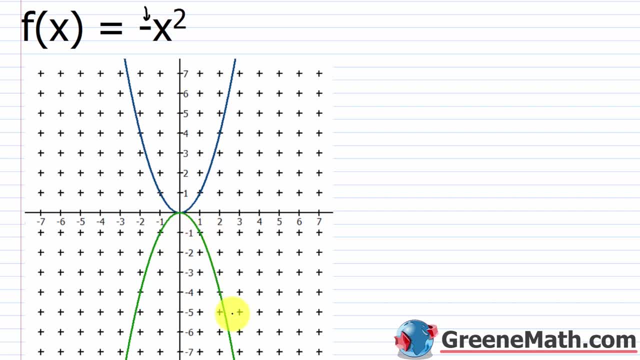 going to have a parabola that opens down, So a downward-facing u. So now, if you think about the vertex, it's going to be the highest point, Right? So this 0 comma 0 here is the lowest point for the upward-facing parabola, but the highest. 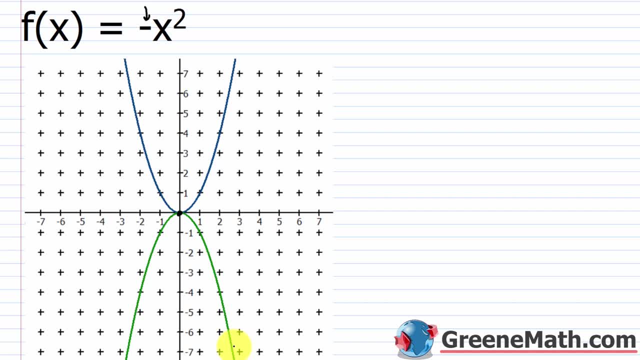 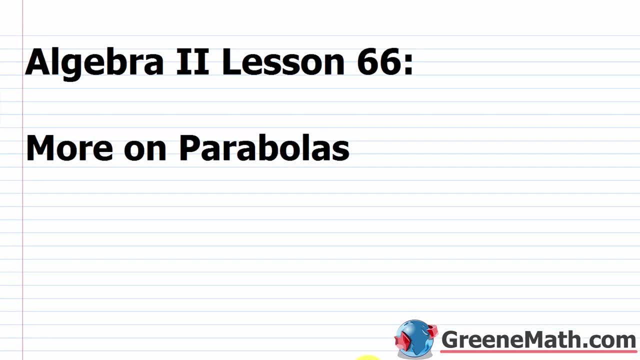 point for the downward-facing parabola. Okay, And as you move higher in math, you're going to start talking about these as minimums and maximums. But again, we'll get to that later on. Hello and welcome to Algebra 2, Lesson 66.. 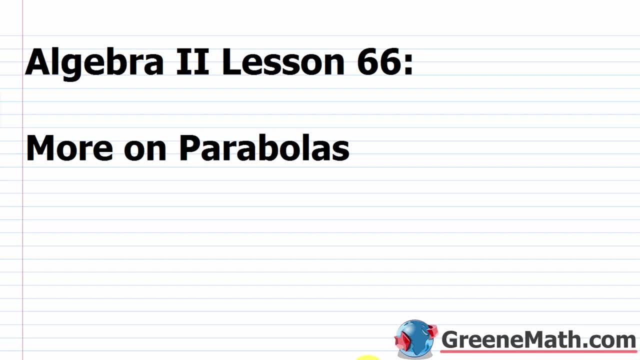 In this lesson we're going to continue to learn about parabolas. So in the last lesson we covered some basic topics that come up when working with parabolas. In this lesson we're just going to go a little bit further and expand on what we know. 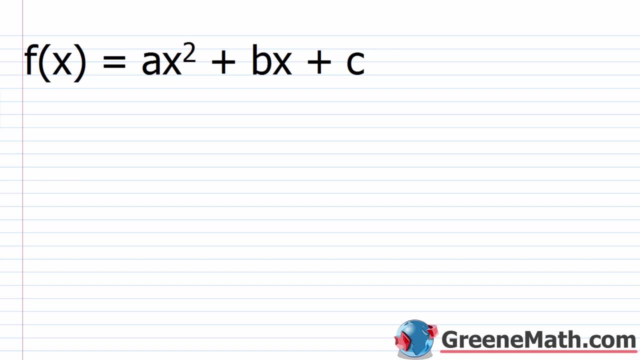 So the first topic we're going to talk about today would be how to find the vertex when our function is in standard form. So we see we have: f of x is equal to ax squared plus bx plus c, and of course here a does. 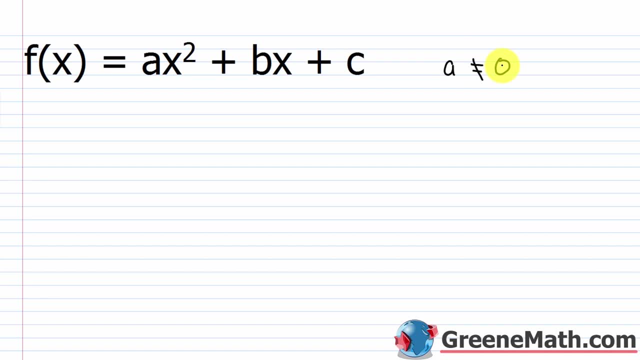 not equal 0.. So what's the vertex here? And, in case you didn't watch the last lesson, what is a vertex in general? So, with a parabola, with a standard parabola, a u-shape that opens up- we know that the 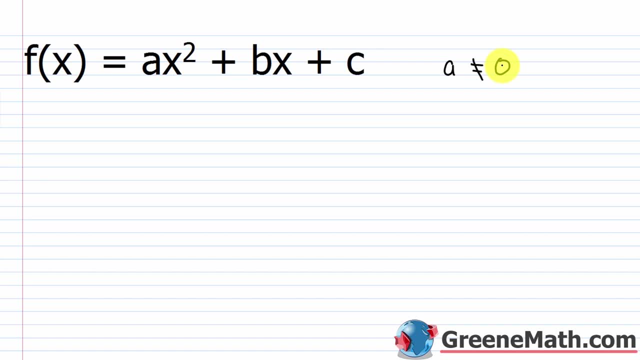 vertex is the lowest point on that graph. So in terms of the y location or the y value on that coordinate plane, it is as small as it's going to get. Now, if you have the other scenario, if you have a parabola that opens down, so an upside- 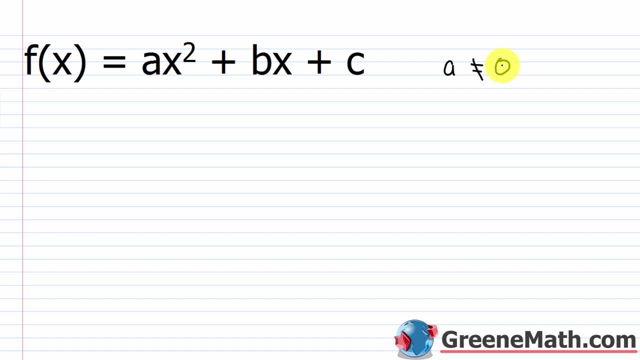 down. u is what that looks like. in that case the vertex is the highest point, So in terms of the y value it's as high as it's going to get. But either way, we use the same formula to obtain the vertex. 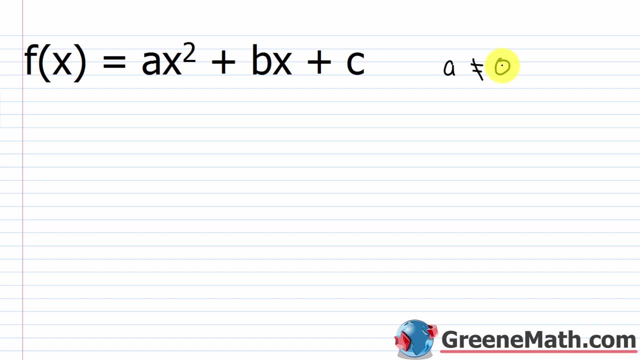 Now, in the last lesson I talked to you about the vertex's slope, Okay, about the vertex form. So vertex form looks like this: It's f of x is equal to. you have a times the quantity x minus h. this is squared, and then plus k. So the reason we call this vertex form is: 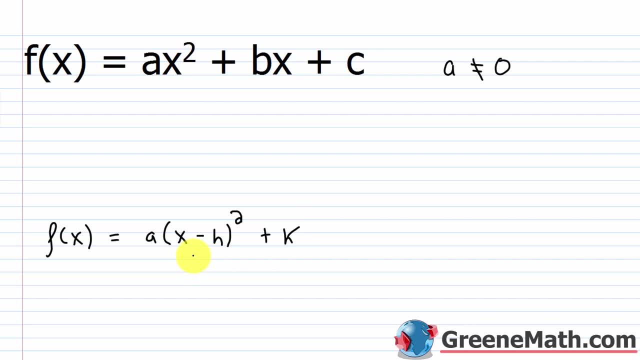 that I can look at this function in this form and I can immediately tell you what the vertex is. So the vertex here? the vertex will occur at the point h, comma, k, meaning whatever is here for h will be plugged in for the x coordinate and whatever's here for k will be plugged in for the. 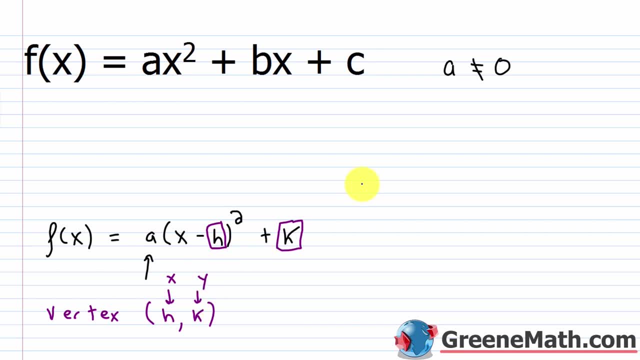 y coordinate. Now, before we go any further, let's think about why the vertex occurs at the point h, comma k. Although you would use the same thought process either way, I want you to think about the fact that if you have a vertex form and you have a vertex form, and you have a vertex form and you 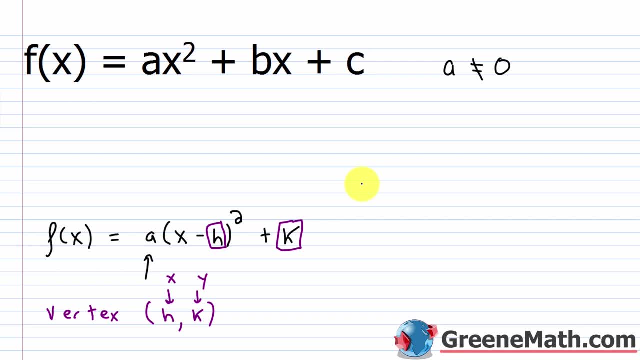 if you had an upward facing parabola, so a standard u-shape, your vertex is going to occur at the lowest possible point, So the y value is as small as it's going to be. So just for a second, replace f of x with y, so we can get past that mental roadblock. And I just want you to think. 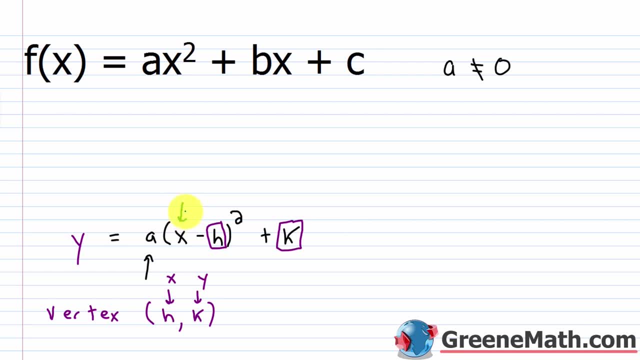 about what you could plug in for x to make y as small as it could be. Well, because we have this squared right here. no matter what I plug in for x, I subtract away from the x coordinate and I get the y coordinate. So if I plug in for x, 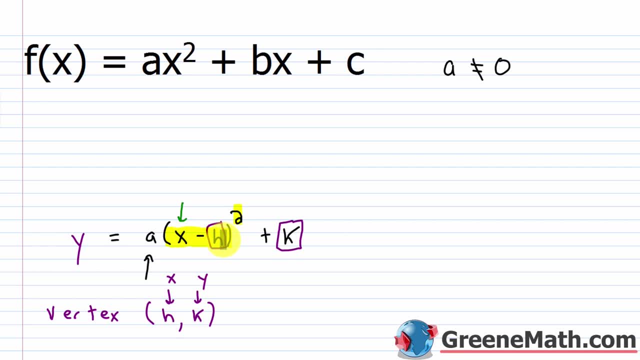 something for h. when I square that, it's going to either be zero or positive, right? If it turns out to be negative when I square it, it's positive. If it turns out to be positive when I square it, it's still positive. If it's zero and I square it, I get zero. So 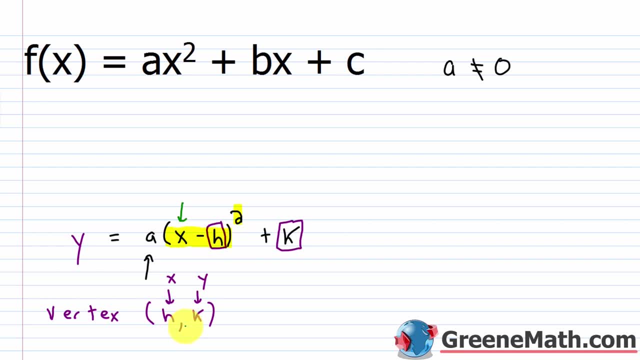 the best I can do at making this small is to plug in an h, right, Because h minus h would give me zero. So this guy right here, once I square, zero would be zero. I multiply it by a, I still have zero. So this is knocked out and I'm just left with k. So that's why your vertex occurs at the. 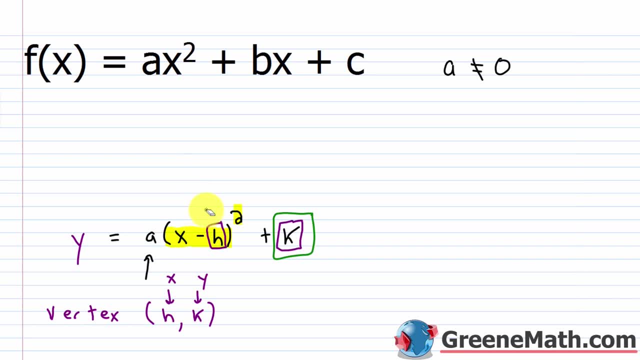 point h, comma k. So now, once we know that, let's think about how we could take a function in standard form like f of x equals ax squared plus bx plus c, and transform it into vertex form. Well, what we're going to do is we're going to use that method known as completing the square. 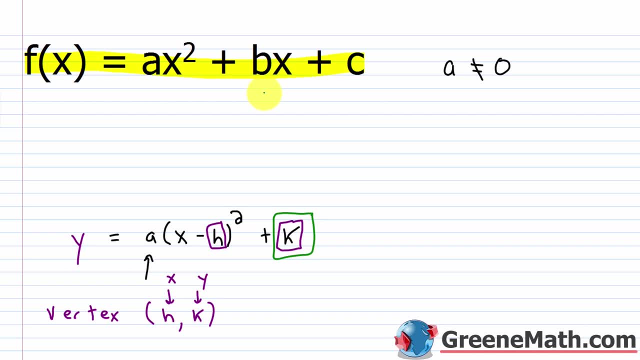 And most of you remember this from when we solved quadratic equations, We saw that we had to start out by learning the square root property, Then we learned how to complete the square, And then we found a shortcut known as the quadratic formula. It's going to be the same thing. 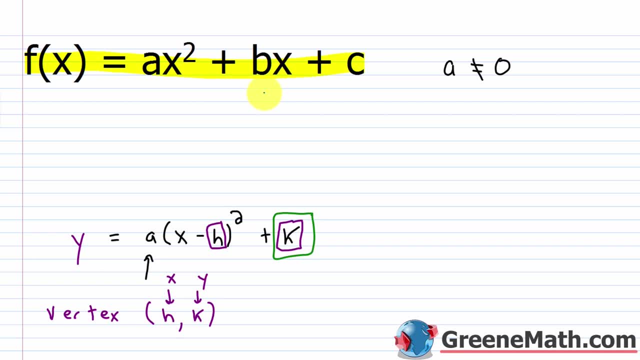 here We're going to complete the square. Then we're going to see a shortcut known as the vertex formula. Okay, so let's jump in and look at an example. So let's say we see, f of x equals x squared minus 9x plus 7.. And your question here is to find out what is the vertex. So, in order to 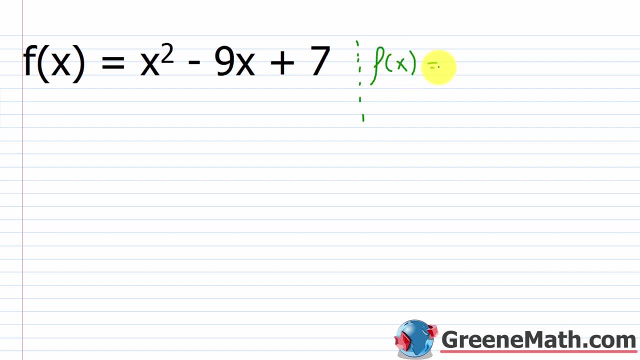 write that form first. so this is: f of x is equal to a times the quantity x minus h squared plus k. All right, so if you remember, from completing the square we start out by moving all the variable terms to one side and all the numbers on the other side. In this particular case, we're not going to. 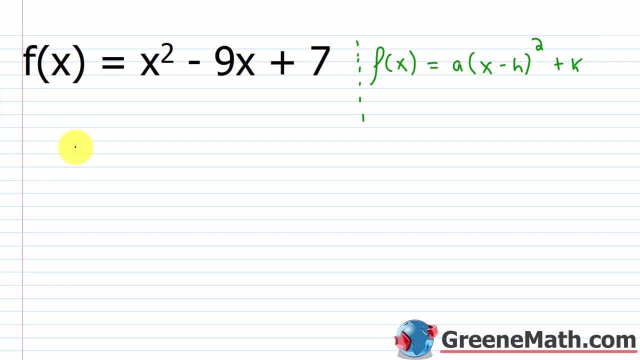 do that. We want to just keep f of x on one side of the equation by itself. So we're not really going to mess with the left side at all. So we're going to start out by moving all the variable terms to one side and all. We're just going to do everything to the right side. But I'm still going. 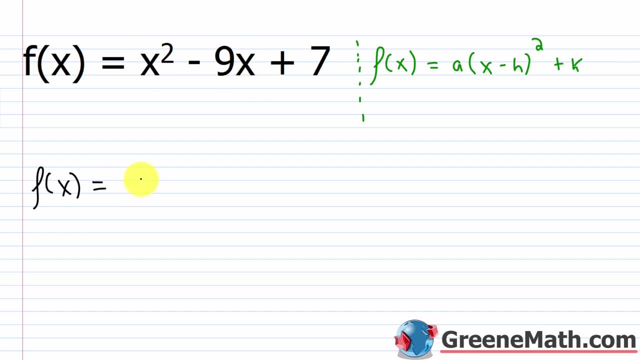 to group the variable terms together. So I'm going to say x squared minus 9x. I'm just going to put some parentheses around it to say this is grouped together And then we have this plus 7.. Now to complete the square. you look at your coefficient for the variable raised to the first power In. 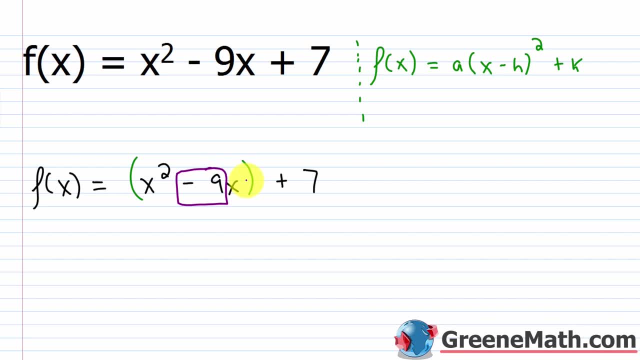 this case, that's going to be negative naught. So what do you do? You cut it in half, meaning you multiply by half, and then you square it. So I would have negative naught and then I would have negative 9 multiplied by a half, And then the result of this is going to be squared. So this: 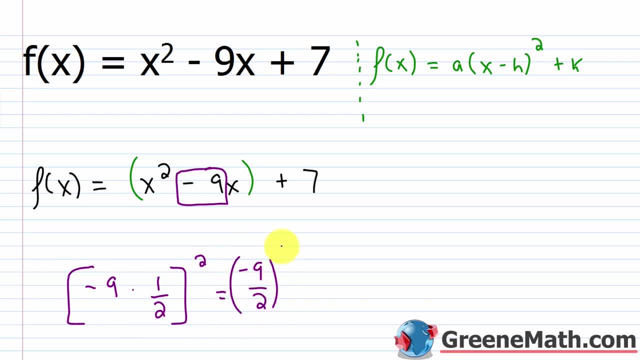 would be negative: 9 halves squared, which would be 81 fourths. Now, what does this do, this 81 fourths? Let me just jog your memory here. So let me erase this real quick, And I'm just going to. 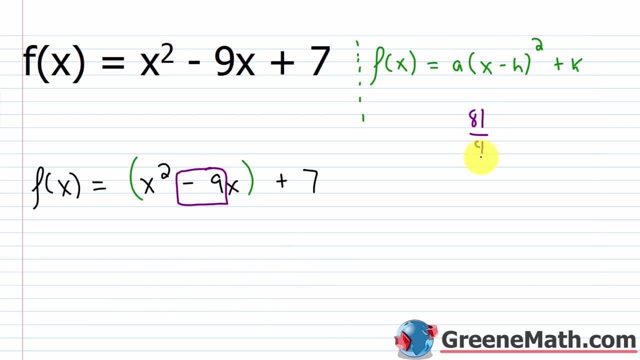 put this value off to the side for a minute. So 81 fourths- The 81 fourths is added right here. That is the constant that makes that trinomial into a perfect square trinomial. So remember, a perfect square trinomial. 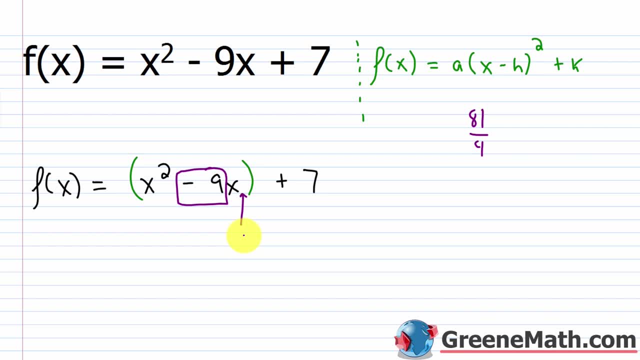 is able to be factored into a binomial squared. That's what we got to get to to get this guy right here. We want a binomial squared, So let's just go ahead and do that, So we would have f of x. 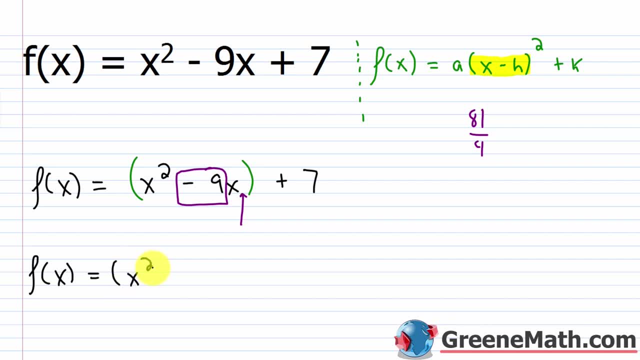 is equal to. we'd have the quantity x squared minus 9x, And then this guy right here is what I'm adding: So plus 81.. So now I've got my perfect square trinomial. But there's a problem. I can't just go around adding. 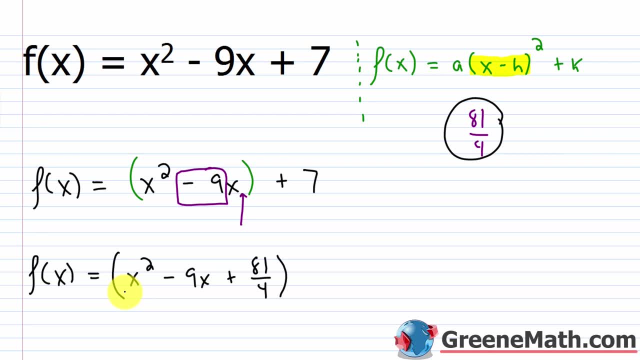 things to equations. right, It's got to be balanced. Normally, if we add something to one side, we've got to add it to the other, But in this case I told you we're not going to mess with the left side of this equation, So what we're going to do is we're just going to subtract it. 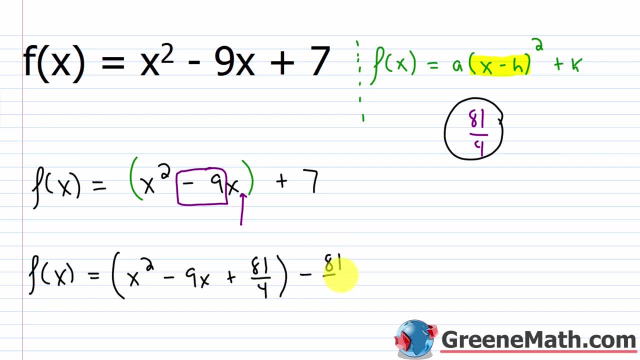 away outside the parentheses. So minus 81 fourths, And then I have my plus 7.. So this right here is going to be a perfect square trinomial. What I'm going to do is I'm going to go ahead and subtract. 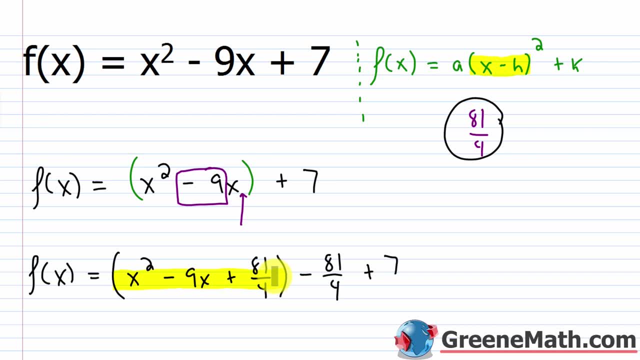 this and add it to my binomial, And this is what I'm going to do here- is I'm going to add a half of this to my binomial squared, So I've got my binomial of x squared. That's my perfect square. 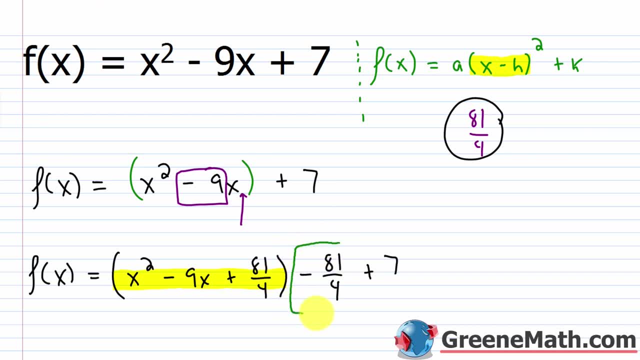 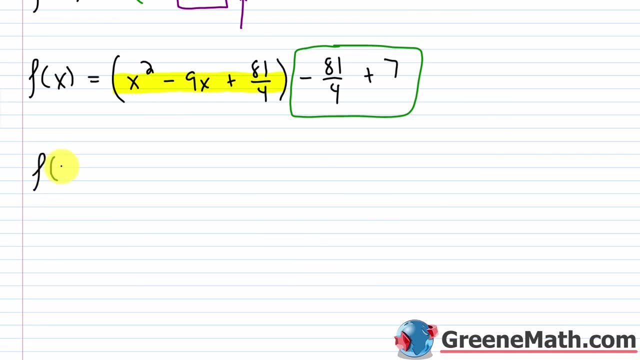 trinomial And then this part right here we can basically say: this is together. So let's scroll down and get some room going, We'll see what we get. So we have f of x is equal to. most. of you remember from special products how to factor a perfect square trinomial. You know that this would 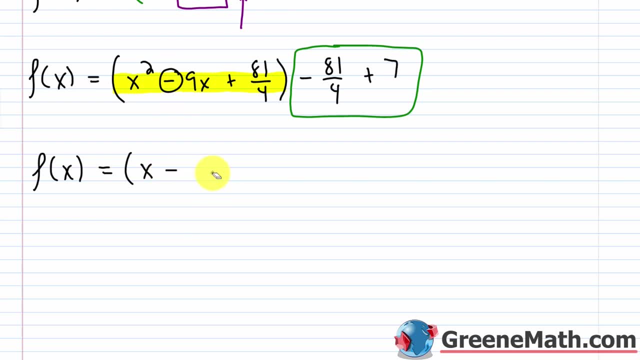 be x. you have a minus here, so you get a minus here, And then you can always take this last term, the square root of it, And so the square root of 81 is 9.. The square root of 4 is 2.. So you get. 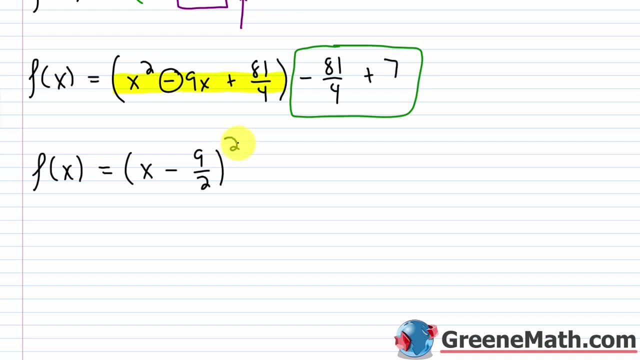 x minus 9 halves. That quantity is squared. And again, if you don't believe that that factors into that, pause the video. do FOIL, you'll get this back. Then we'll have minus 81 fourths and then plus 7.. Now I want to combine these two, So I want to get a common denominator going So. 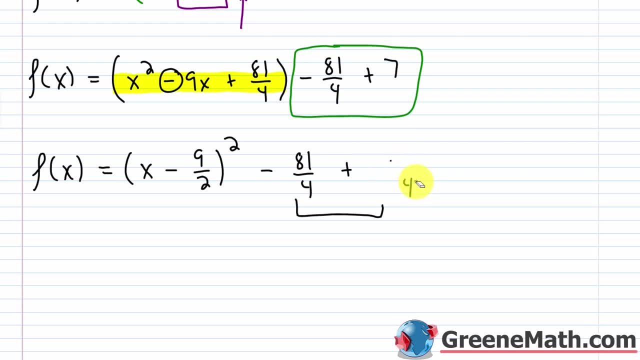 I multiply this by 4 over 4.. 7 times 4 is 28.. So you would have 28 fourths there, And then now it's just a matter of adding negative 81 and 28. So if we do that, we get negative 53.. 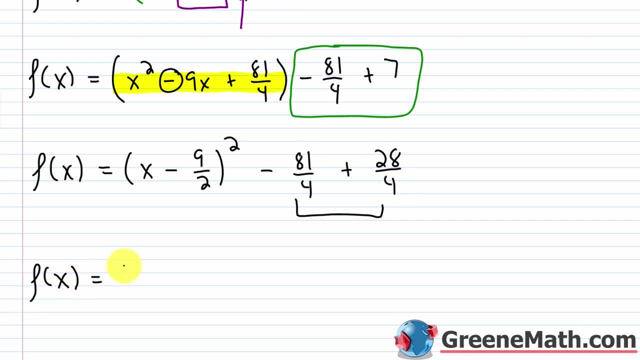 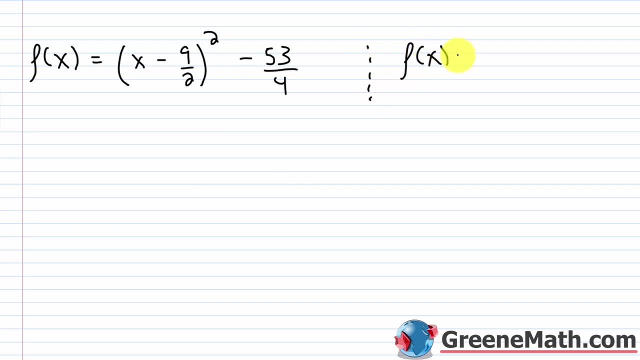 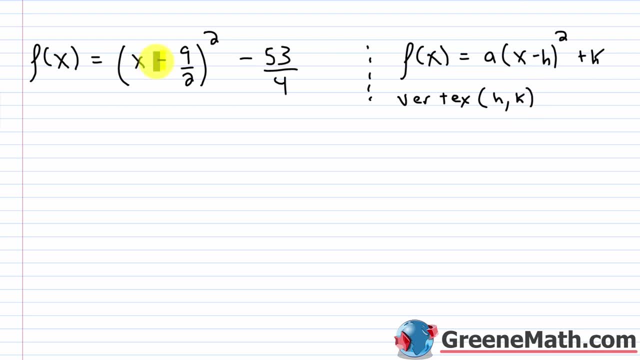 careful. You do have a minus sign here and here. So whatever occurs after that minus sign, in this case that's going to be your x coordinate for that ordered pair. So the vertex, the vertex occurs at the point. you'll have 9 halves, But then you have a plus sign here but a minus sign. 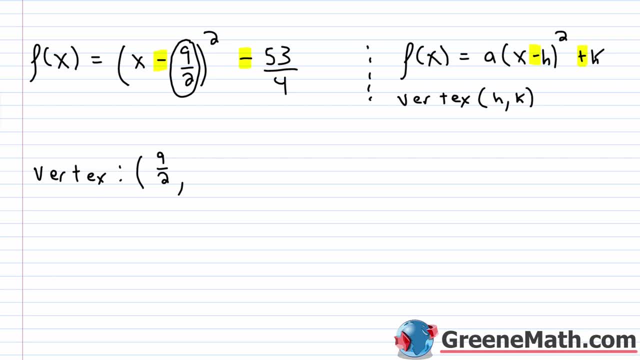 here. So you've got to be very careful. Go ahead and translate this into plus a negative 53 fourths, So you don't make a mistake. And so negative 53 fourths represents k, So that will be your y value. So negative 53 fourths, So the vertex for this function is going to occur at the point 9. 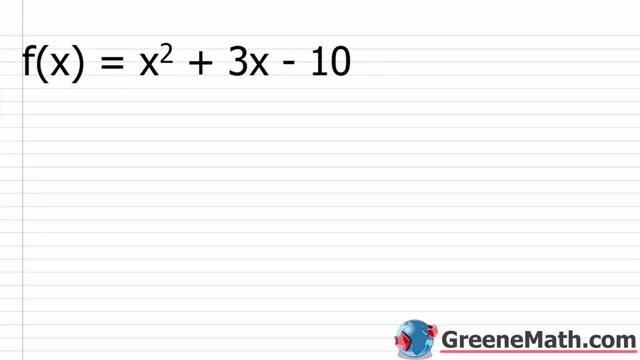 halves comma negative 53 fourths. All right, let's try another one now. So we have: f of x is equal to x squared plus 3x minus 10.. And again, I want to put this in vertex form. So for vertex form. 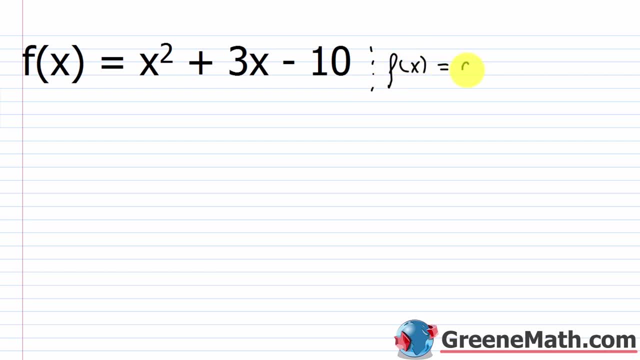 it's f of x is equal to a times the quantity x minus h. This is squared. then plus k, Now the vertex. again, the vertex will occur at the point h comma k. All right, so let's go ahead and take this guy. we have f of x. 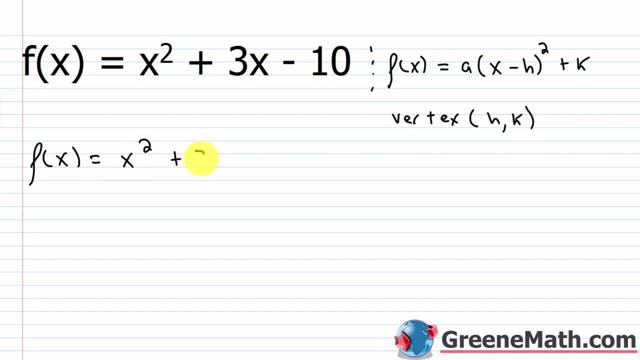 is equal to x squared plus 3x minus 10.. Again, I'm going to group these variable terms together. Normally I would move negative 10 over to the other side by adding 10 to both sides of the equation. But again, if you're doing this, you want to make sure that you have a plus sign. 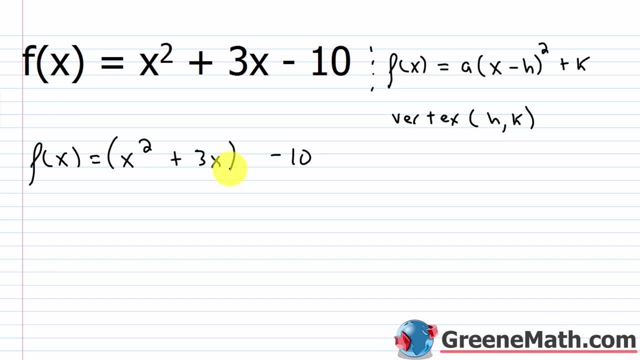 f of x by itself, So I'm just going to leave it alone. I want to add one half of this coefficient right here, which is three squared. So one half times three squared, that would be three halves squared, which would be nine fourths. So I'm going to add nine fourths inside those parentheses. 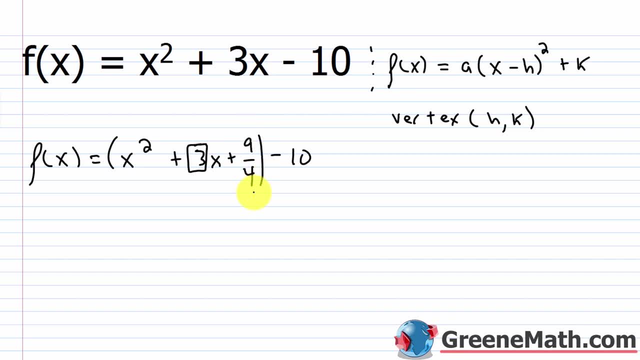 But again, I can't just do that, I can't just go around just adding things to equations. I've got to make it balanced. So I'm going to subtract nine fourths away from the same side of the equation, because nine fourths minus nine 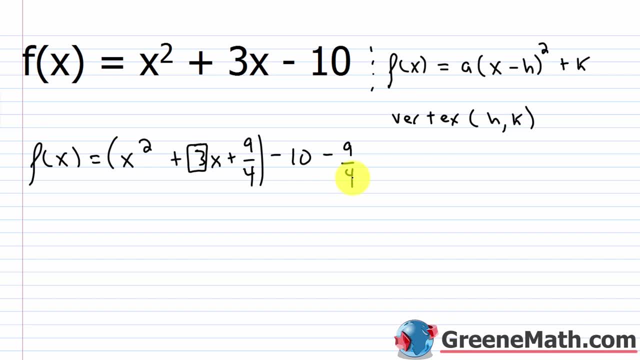 fourths would be zero. Okay, so now that that's done, this can be factored into a binomial square. So we would have: f of x is equal to this would factor into x plus three halves that quantity squared, And then you'd have your minus 10 minus nine fourths. Of course I'd want to get a common 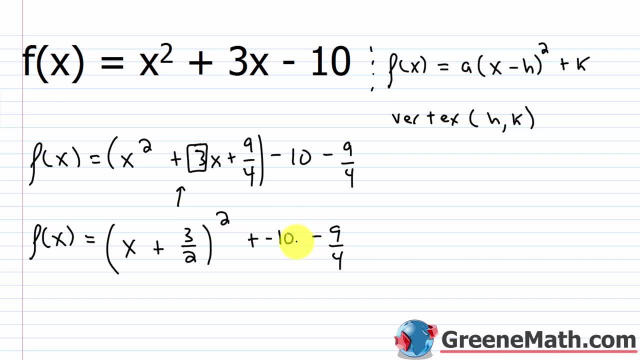 denominator going, So let's put that in there. And then I'm going to add another half of this. This is plus negative 10.. We'll multiply this by four over four, So you'd have negative 40 fourths. So negative 40 fourths minus nine fourths, So you'd end up with minus 49 fourths. 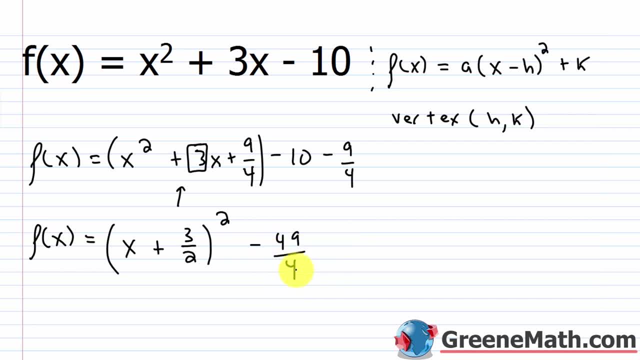 So minus 49 fourths. So we have this in vertex form. But again, you have to be very careful: This is a minus here, This is a plus here. So if you just go through and say, okay, my vertex. 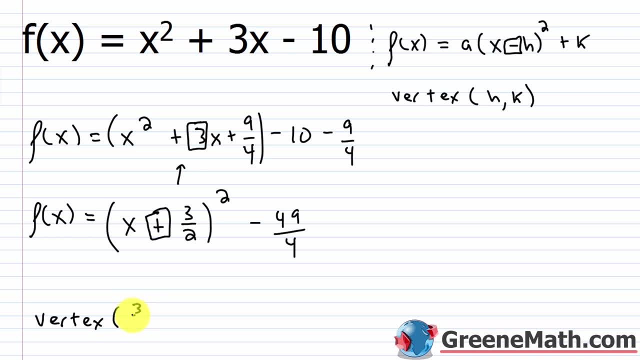 my vertex will occur at three halves, comma 49, fourths. you will be wrong. The signs just won't be correct. So I want to erase this. I don't want to match this up with this. I can make a plus into: 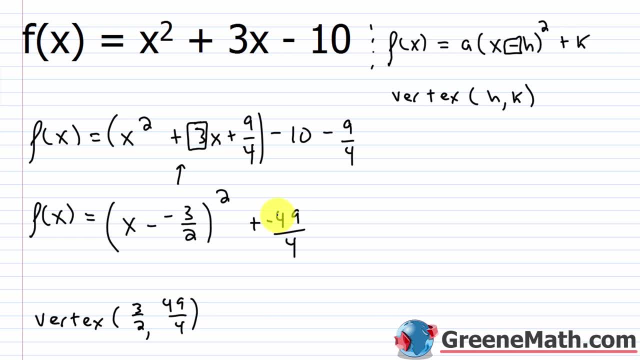 minus a negative And I can make a minus into plus a negative. So now it matches exactly And we'll see that h is negative three halves. So I just put a negative out in front here And we kind of make that a little better. So negative three halves And we'll see that h is negative three halves. 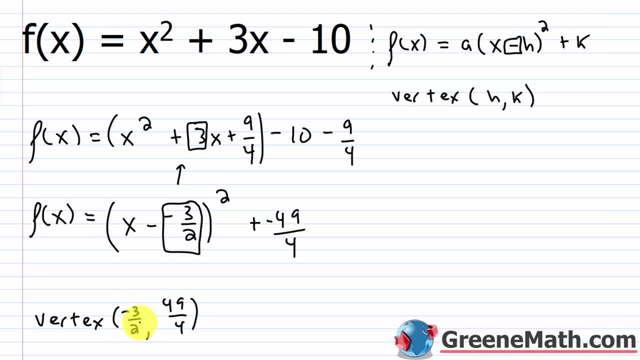 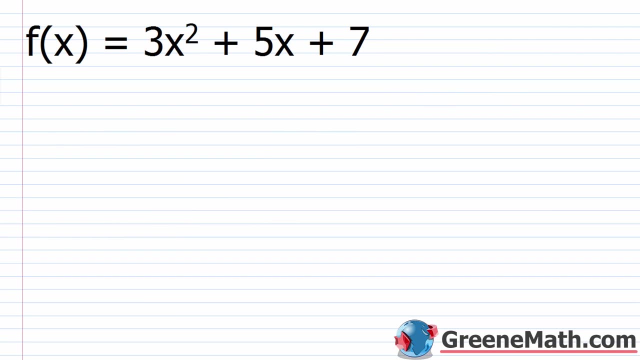 And k. okay, k is going to be negative 49 fourths, So negative 49 fourths. So the vertex here occurs at negative three halves comma: negative 49 fourths. All right, let's take a look at one more of these And then I will show you how to derive the vertex formula. And from: 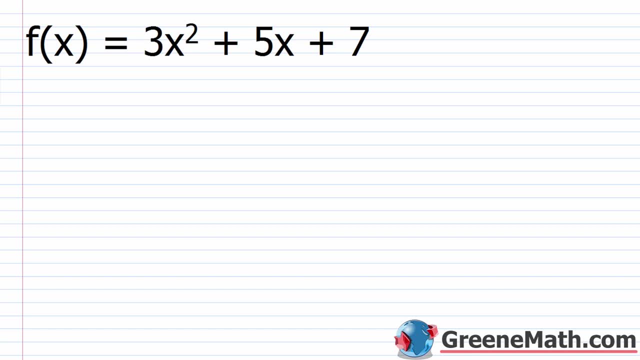 that you will find a very, very easy method to find the vertex when your function is in standard form. So we have f of x equals three. So we have f of x squared plus five, x plus seven. So the one problem here is that we have this three. 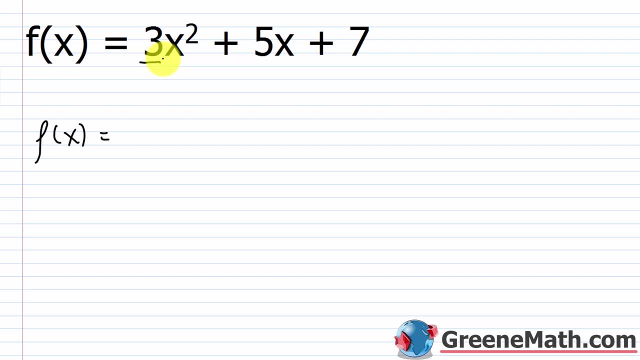 That's the coefficient for x squared. You will recall, when we complete the square, we say that we want the coefficient of the squared variable to be one, right, You'll recall that step from when we completed the square, when we're solving quadratic equations. So what we would. 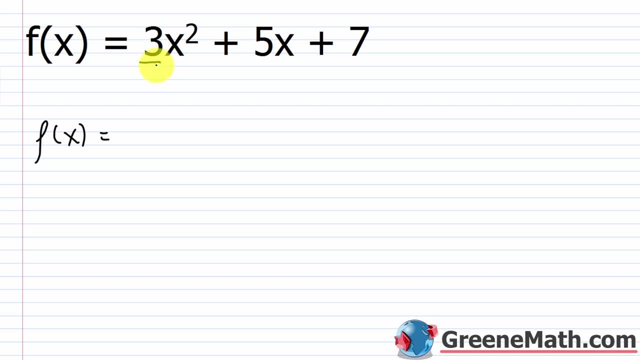 do is we would divide the whole equation by. in this case it would be three. But we're not going to do that here. What we're going to do here is we're going to divide the whole equation by three. We're just going to factor it out from this grouping here. So, in other words, if this is a 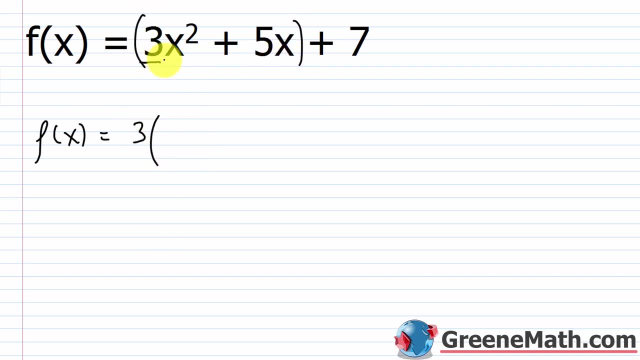 group, I could factor a three out from that group. And if I factored a three out from three x squared, I would have x squared. If I factored a three out from five x, what would I have Five x divided by? 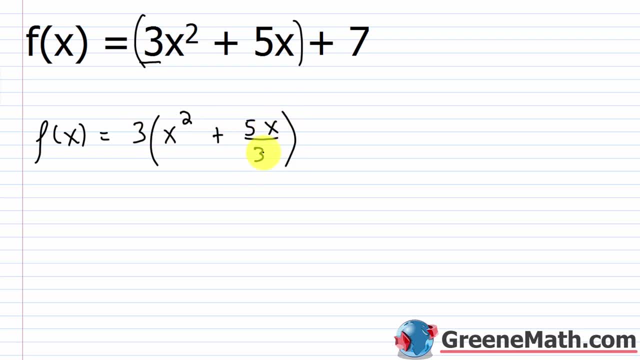 three is what I'm looking for there, Because three times five x over three the threes would cancel and I'd be right back to five x. Then I'd put plus seven and I can kind of move that out And I can go through the process now just completing the square. So I want to take 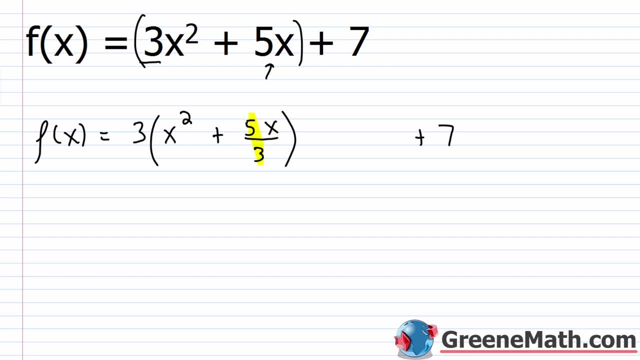 one half of my coefficient for the variable raised to the first power and square it. So five thirds times a half squared. So this would be five sixths squared. Five squared is 25.. Six squared is 36.. So now I want to add 25 over 36 to this side right here. Here's where you have. 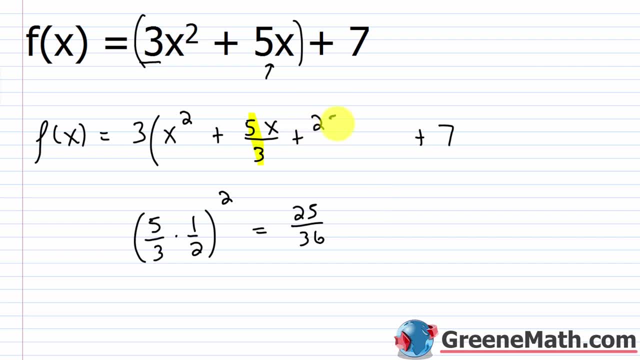 to be careful, though, So I'm going to show you a common mistake. So plus 25,, minus 25 over 36, close the parentheses minus 25 over 36.. So students will do that, and then they'll continue to solve the problem. This is going to give you the wrong answer. Why do you? 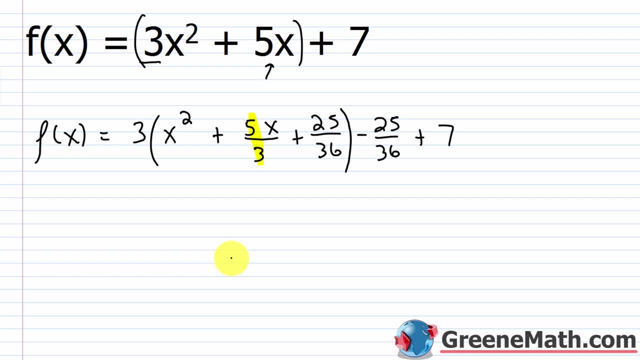 think that's the case, in case you haven't seen it already. Well, you're multiplying three by this guy right here, So I'm not really adding 25 over 36.. I'm multiplying three by 25 over 36.. So I've. 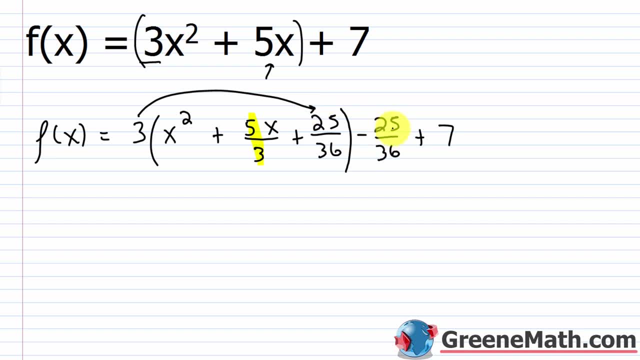 got to do the same thing to this guy, Otherwise I'm not balancing the equation. So I'm going to do the equation. So what I usually do is I'll expand my parentheses out here And then I'll do another step. So I'll do: f of x is equal to three times the quantity, So I'll tighten my parentheses. 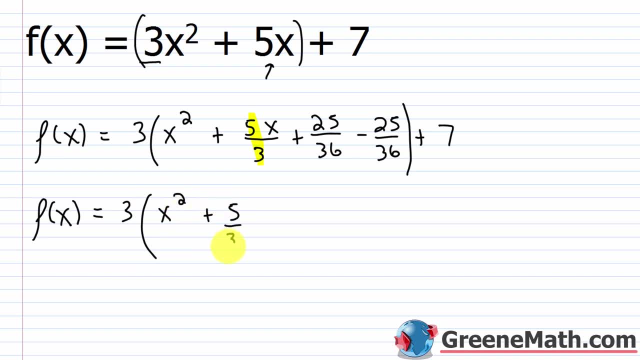 down. I'll say x squared plus five thirds x plus 25 over 36.. I'll close my parentheses there. But this allows me to remember that three is going to be multiplied by this. So I'll put plus negative, 25 over 36.. And then I'll close my parentheses there. So I'll close my parentheses there, And 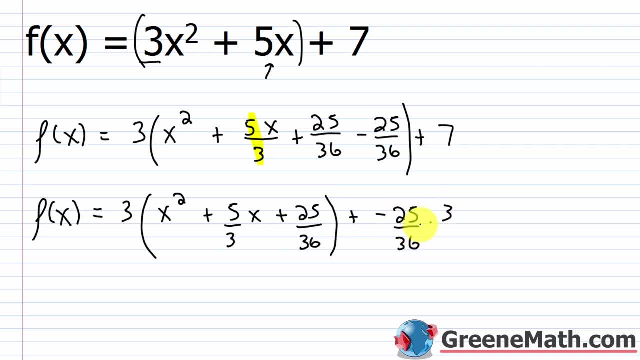 I'll say x squared plus five, thirds x plus 25 over 36 multiplied by three. Now I have added and subtracted the same value to that right side of the equation, So I'm good to go. So then, plus seven. Okay, so let's scroll down, get a little room going. Alright, so we're gonna have f of x. 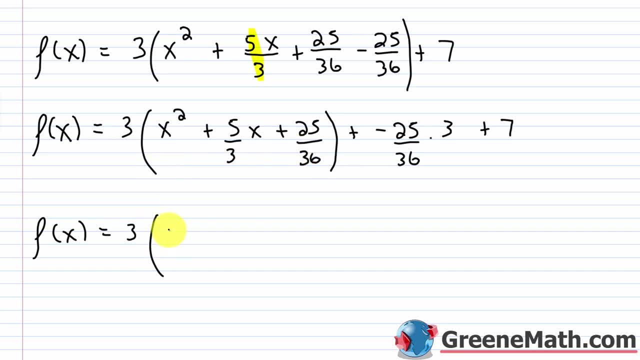 is equal to three times. if I factor this guy, I'm going to have x plus five sixths in this quantity squared. Then over here I have negative 25 times three. that's negative 75. So you'd have to be plus seven. So I would get a common denominator going And to do that I multiply. 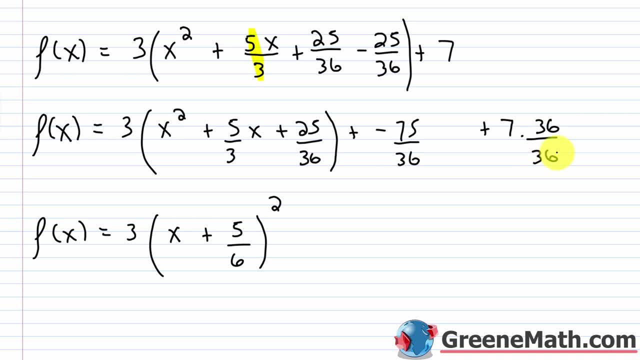 this by 36 over 36.. And so seven times 36 is 252.. So you would have 252 minus 75,, which is 177.. So you could say this is plus 177 over 36.. Now I can reduce this fraction. 177 is divisible by three. 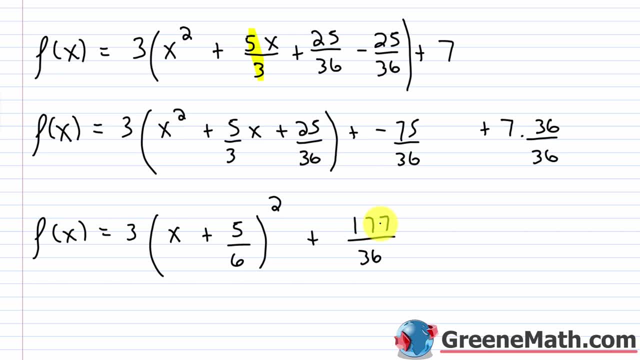 one plus seven is eight. eight plus seven is 15. And so is 36, right? Three plus six is nine. If I divide 177 by three, I get 59. So this is 59. And then 36 divided by three is obviously 12.. Okay, so I have this in vertex form, But again, 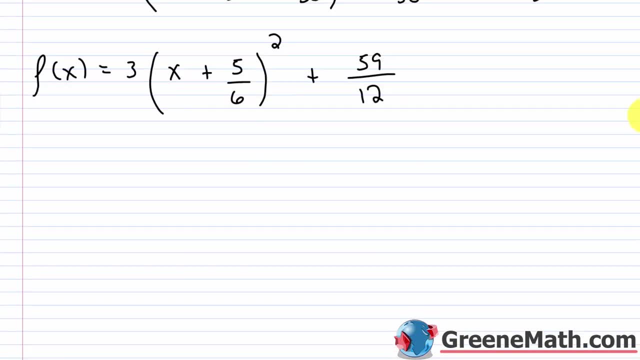 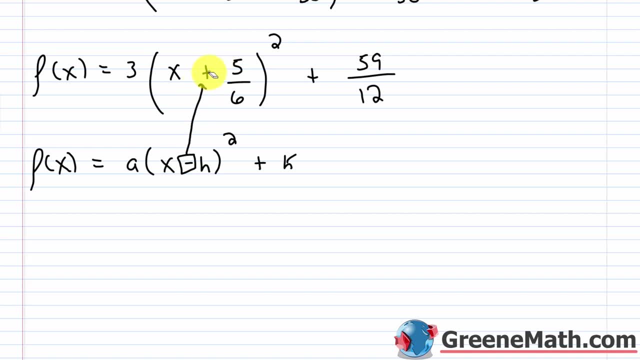 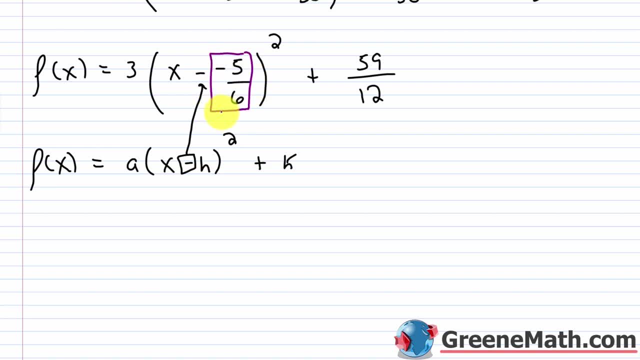 so that this value right here can be plugged in for h. Then I have plus k, So in this case I have plus 59 twelfths. That's okay, right, This will just match up completely. That'll be my value. 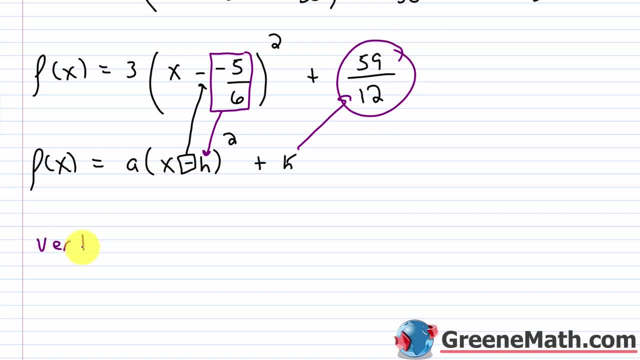 for k. So the vertex, the vertex will occur at negative five, six. That's my h here, And so that's going to be my x value, And then I'm going to plug in my h, And then I'm going to plug in my h, And. then I'm going to plug in my h here, And then I'm going to plug in my h here, And then that's how we're going to convert that value. This is a plus and minus k, And this will find to be my h value. 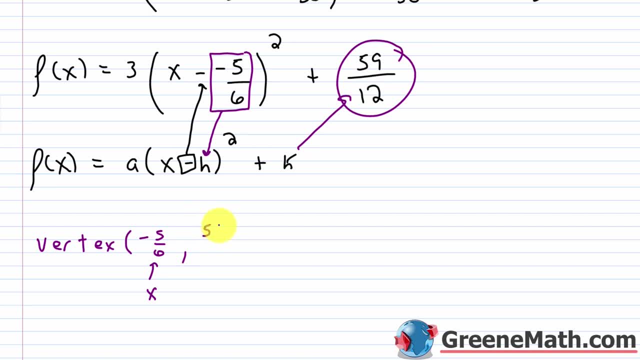 comma k is 59 twelfths, So 59 twelfths will be my y value, So the vertex occurs at the point, at the point negative five, sixths comma 59 twelfths. All right, so now what we're going to. 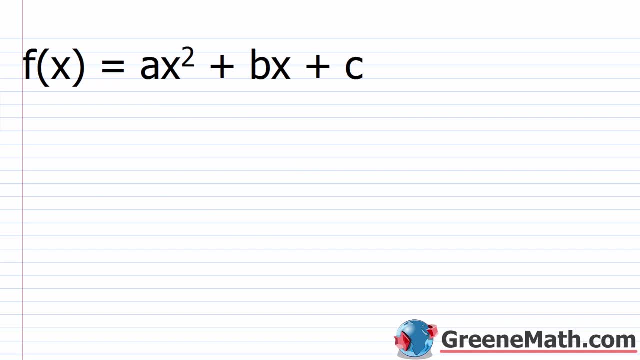 do is we're going to take a generic quadratic function in standard form and we are going to convert it into vertex form And from this we're going to derive something known as the vertex form. So if we convert this into the figure of 1 by 2, and from this we're going to derive something, 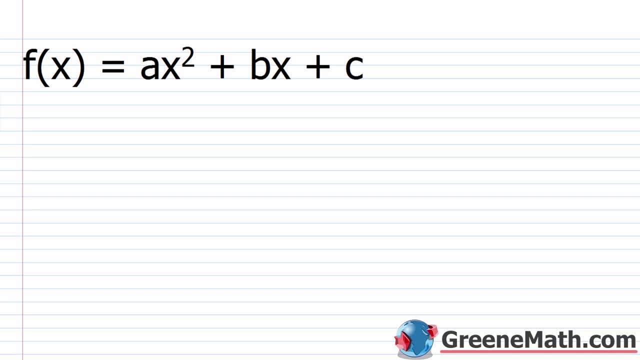 formula. this is basically the same thought process as we use when we derive the quadratic formula. right, we have these parameters a, B and C that we can just easily grab and plug into the formula that we have, and we can solve things very, very quickly. so if I was to have this guy right here and again, I 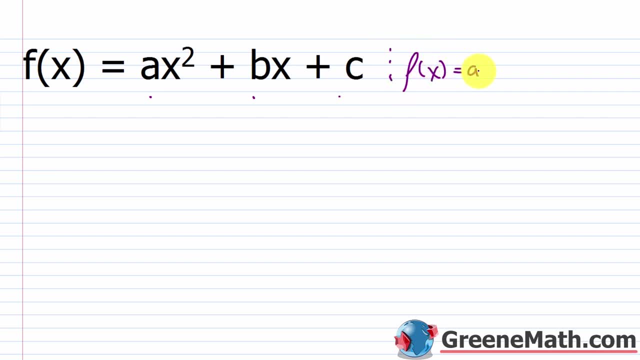 want this in the format of f of X is equal to a times the quantity X minus H squared plus K. the first thing I would do is I would factor out the a from these first two terms right here. so f of X is equal to bring the a outside I. 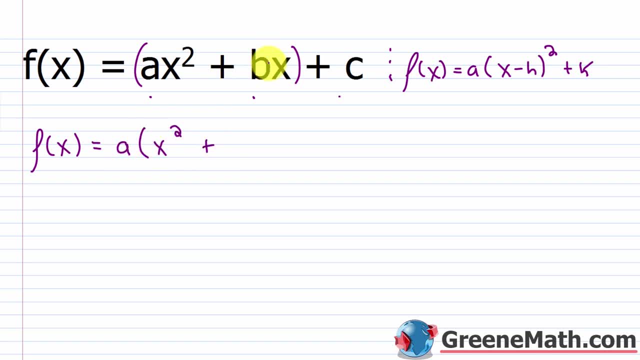 would have x squared plus. so factor an a out from here. I would basically divide B times X by a. so in other words, this would be B X over a, and again, if a multiplied by B X over a, the a's would cancel, be back to B X. so then we can close this and then we'll. 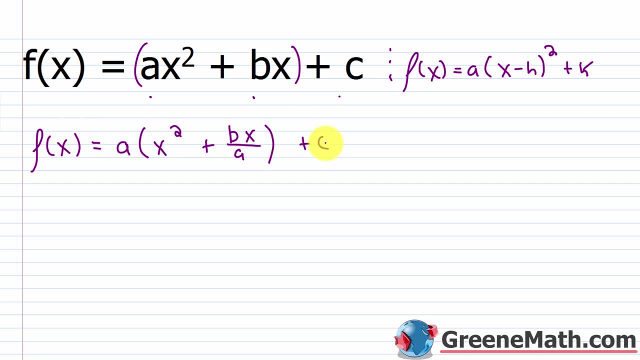 have plus C, okay. so now that we've done that, we want to complete the square. we want to take this guy right here and just make it into a perfect square, trinomial, so that we can factor it into a binomial square. okay, that's the goal. 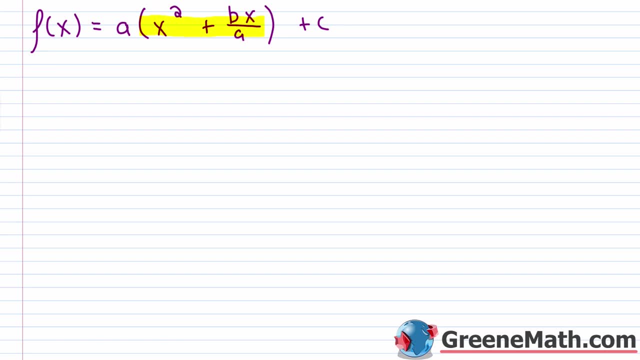 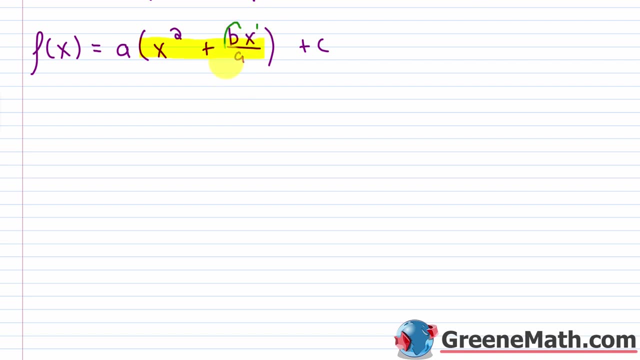 so let's scroll down, get a little room going, all right, so I want to take my coefficient for the X to the first power variable. in this case that's going to be B over a, so B over a, and I want to cut it in half. so multiply by half and then I 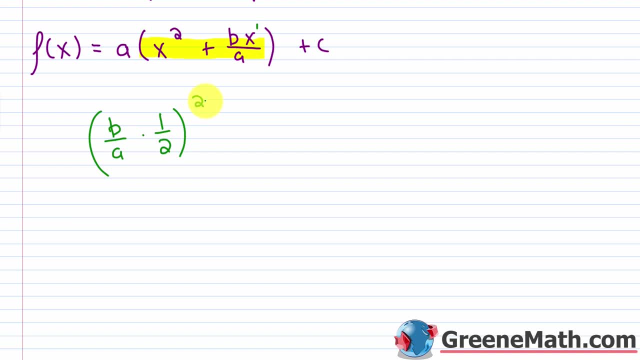 want to square the result, so this would be B over 2a, so this would be B over 2a and this would be squared, giving me B squared over 4 right. 2 squared is 4 times a squared. okay, so now let me erase this and let me kind of scooch this up again. 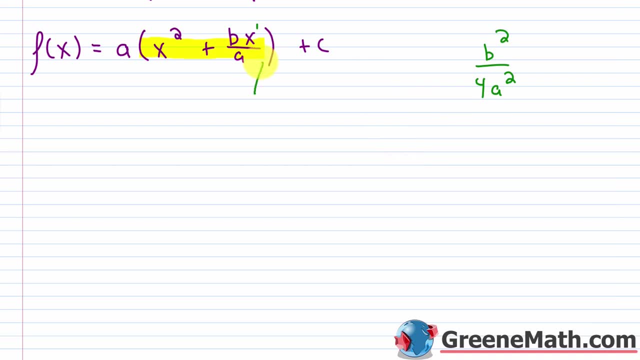 let me erase this and let me kind of scooch this up again. let me kind of scooch this up again. we have to be careful: if I just shove this in right here, remember a is going to be multiplying by that, so I can't just balance it outside of the. 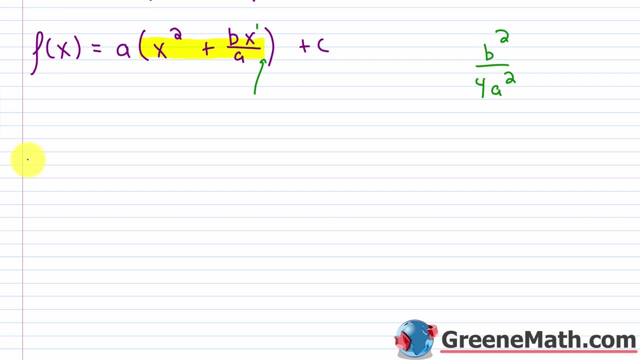 parenthesis. okay, so what I want to do- to remind myself, I'll have f of X is equal to a times the quantity x squared plus B over a, X plus B squared over 4a squared. then I'm going to put minus B squared over 4a squared. this is all in the 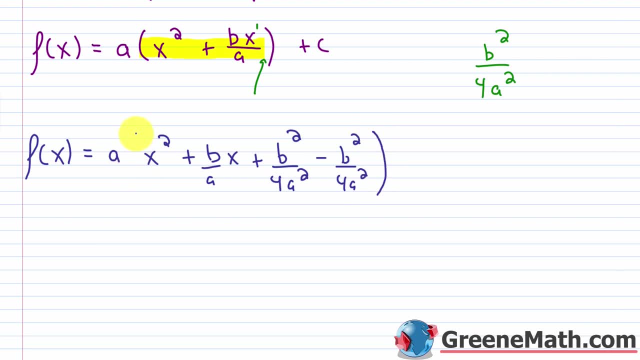 inside the parenthesis, then I'll close the parenthesis. okay, right now, the way it's set up, a would multiply all of these, so I am adding and subtracting the same value to the same side of the equation, and so I'm basically adding 0, right, I'm? 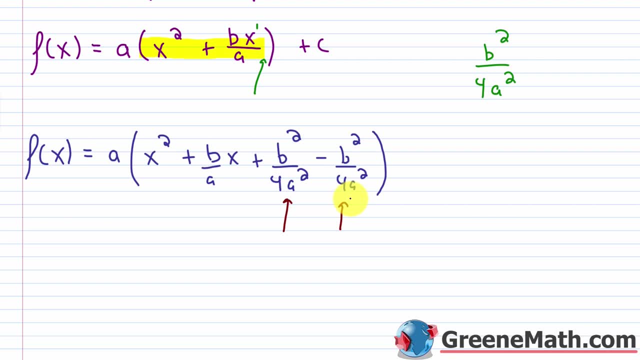 not changing it. it's balanced. okay, that's what you have to do. if you make the mistake and you do this and you forget to multiply by a, you're gonna get the wrong answer. so make sure you put your parentheses here as a reminder, and then we'll see you in the next video. 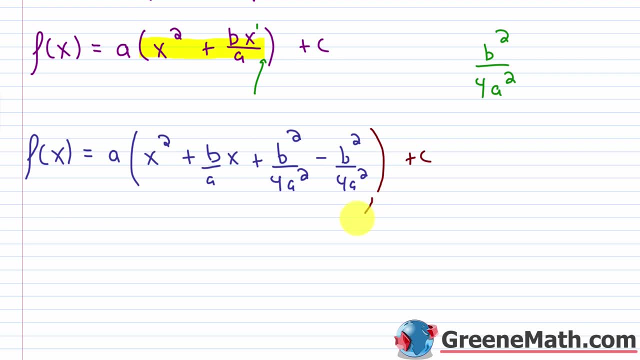 we'll put plus C here. now, in the next step we'll tighten this down. but the way we're gonna do it, we're gonna say f of X is equal to a times the quantity x squared plus B over a. X plus B squared over 4a squared. I'll close the. 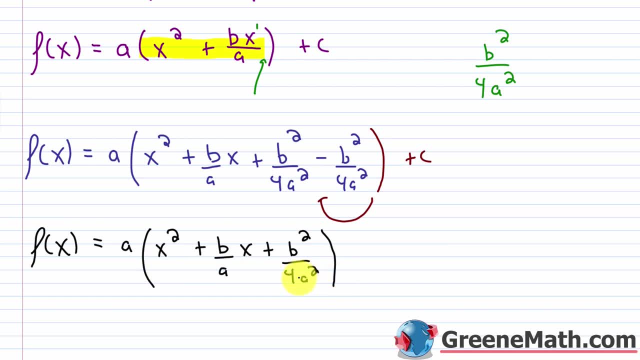 parentheses, because this is a perfect square trinomial. but then I'm going to remember that a is going to need to be multiplied by this negative B squared over 4a squared. so plus B squared over 4a squared, plus B squared over 4a squared. 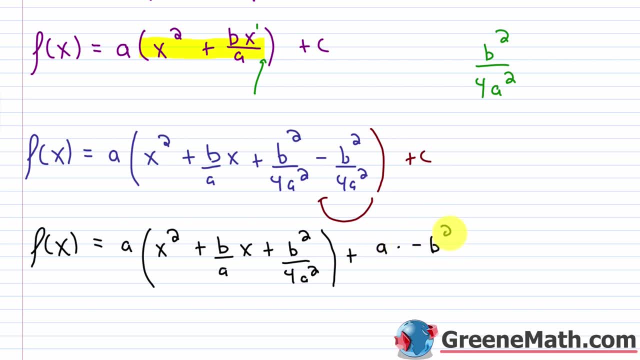 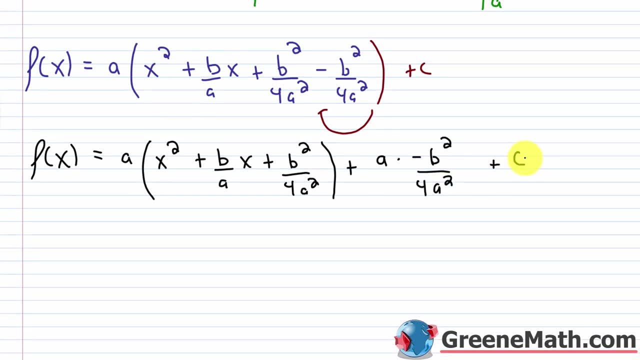 plus, we'll have a multiplied by negative B squared over, 4a squared. scroll down, get some room going. and then of course, we have plus C. okay, so now we have a perfect square trinomial here, so I'm gonna factor that guy into a binomial. 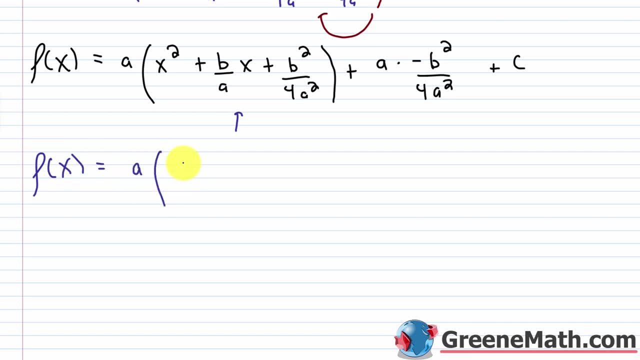 square, so f of X is equal to a times the quantity. this would be X plus square root of B squared is B. square root of 4a squared is 2a. and then this quantity is squared then plus over 2, cause b squared over 4a squared is 2a squared. so then what we end up. 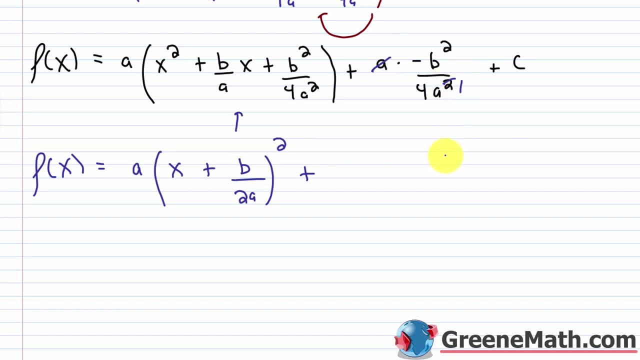 doing over here. I just need to do some simplification, so this would cancel. with one of these I'd have negative B squared over 4a. now I can flip this around and say I have see-b squared over 4a, and then I can get a common denominator buy. 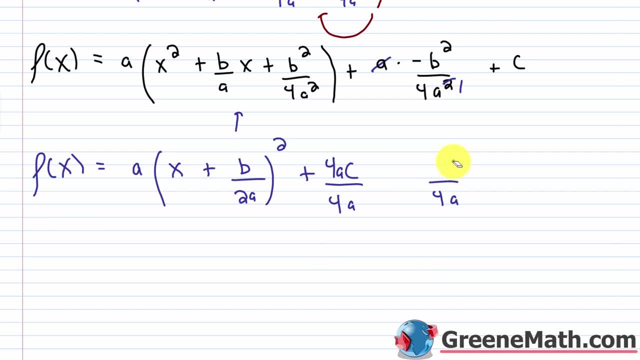 multiplying this by 4a over 4a and what's gonna end up happening is I have plus 4ac minus b squared, so 4ac minus B squared over the sum that's being calculated here, boiling in the description below, where you'll find that there was one específic form over for a. 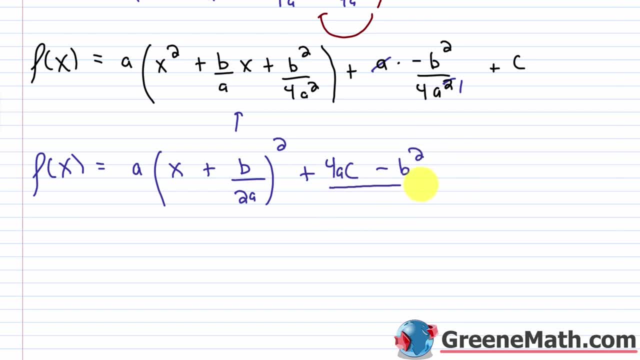 over the common denominator of 4a. Now there's one other thing we want to do here. Remember when I show you vertex form. it's: f of x is equal to a times the quantity x minus h squared plus k. So here k is this guy right here? 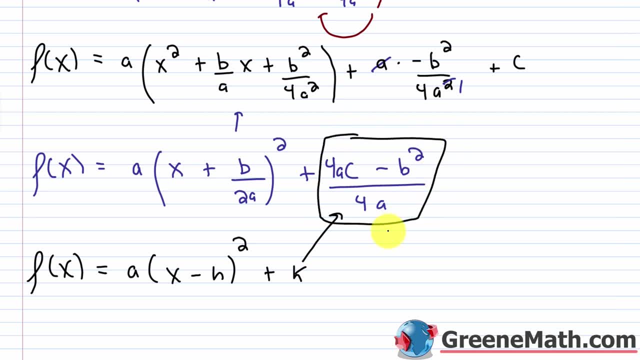 So that's going to be the y-coordinate when you're talking about your vertex, And then h. there's a problem getting it straight from this because you have a plus sign here and here you have a minus. So we want to just make one minor change here. 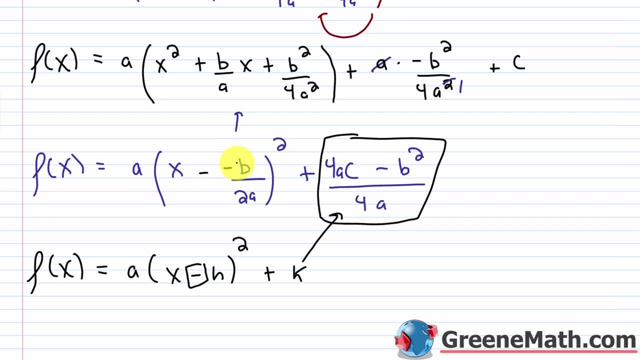 and put this as minus a negative b over 2a. And now this guy right here will be my h. That's what's going to get plugged in for my x location when I'm building the vertex, But it's going to get even simpler than that. 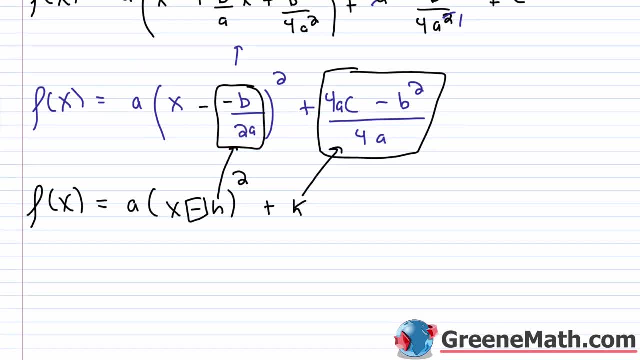 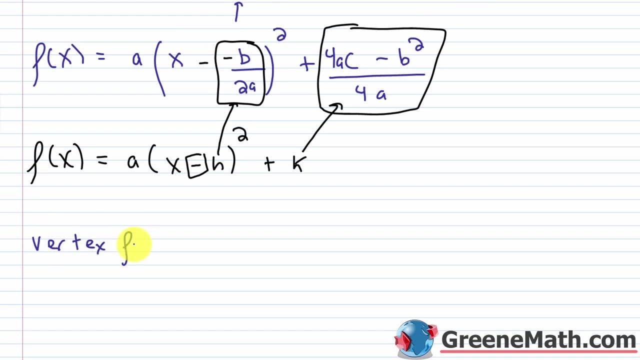 So let's scroll down just a little bit And let's write our vertex. So this is the vertex, This is the vertex formula, And you definitely want to write this down because it's going to save you a lot of time. So the vertex formula: you take a quadratic function in standard form. 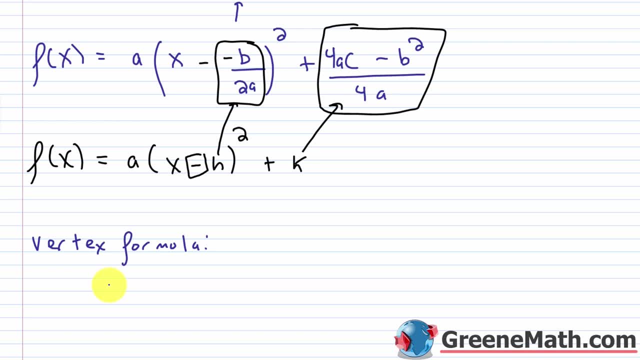 and you know what a, b and c are And you can plug into this formula and find out the vertex. So the vertex will occur at the point negative b over 2a, And that came from right. here again, Normally it's h. 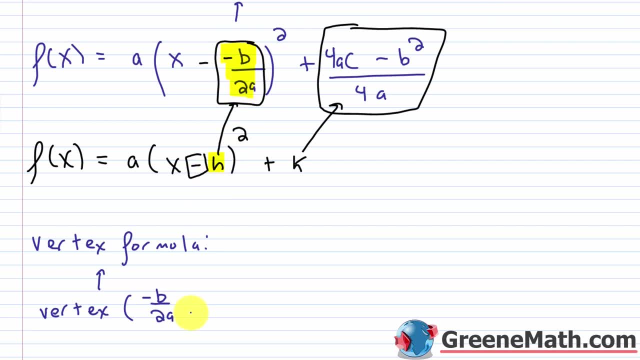 h. here is this: negative b over 2a, Then comma. you could plug in 4ac minus b squared over 4a. But there's an easier solution. I want you to think about the fact that if I plugged in a negative b over 2a for x, 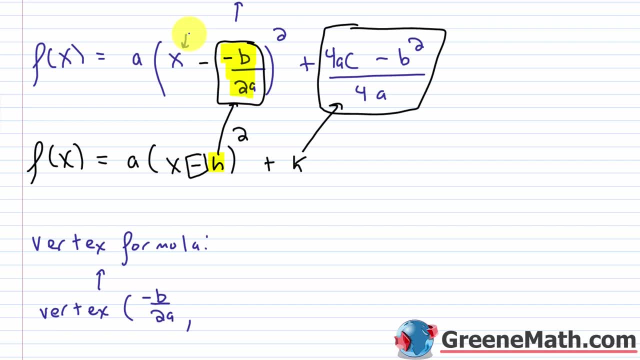 what would happen there? Well, you would get zero, And again this would cross itself out. You'd just be left with this. This is what would be left. So, instead of, Instead of writing all this, all I want to say is that I want to plug this in for x. 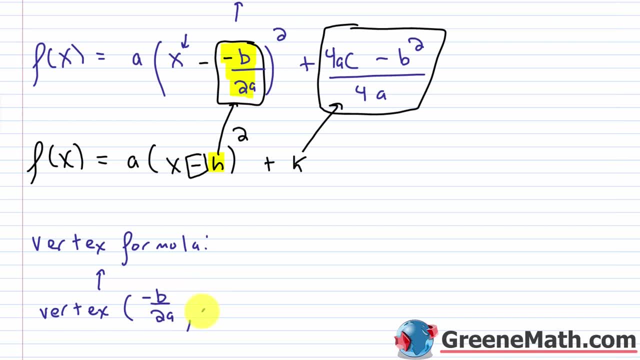 How do we do that with function notation? Well, we say f of whatever we want to plug in for x. So in this case that's negative b over 2a And that's going to be my value for y, or you could say your value for k. 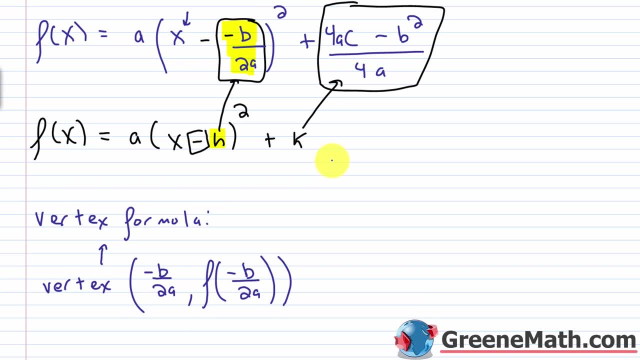 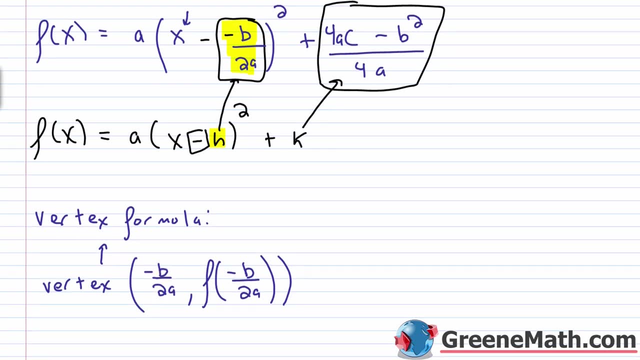 however, you want to think about this, So hopefully that makes sense for you. Again, the vertex formula: the vertex occurs at the point and negative b over 2a. this is what's going to be the x location on the coordinate plane. 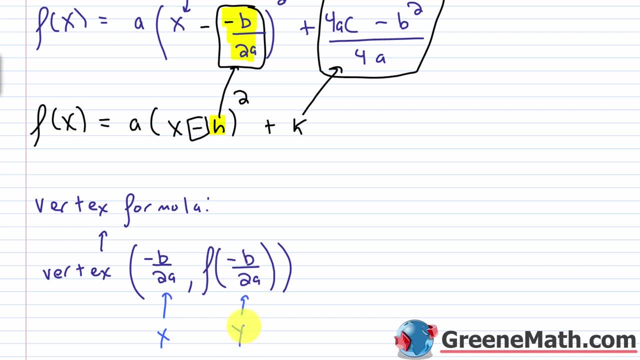 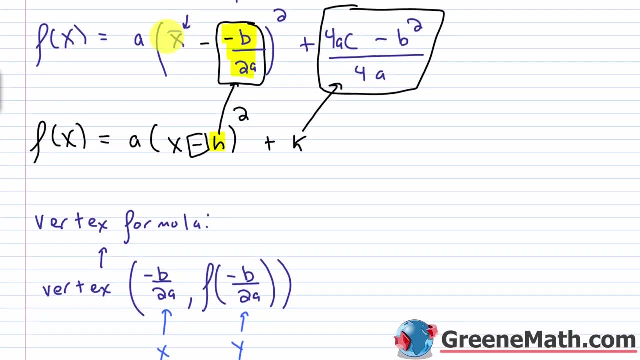 And then f of negative b over 2a. this is your y location on the coordinate plane. And again, just so you're not confused, the way we got that is, if I plugged in a negative b over 2a in for x, this part right here would go away. 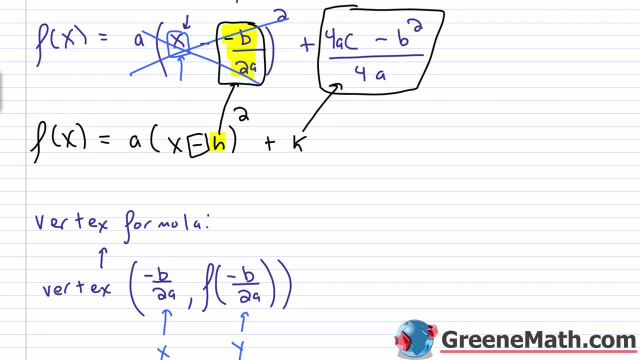 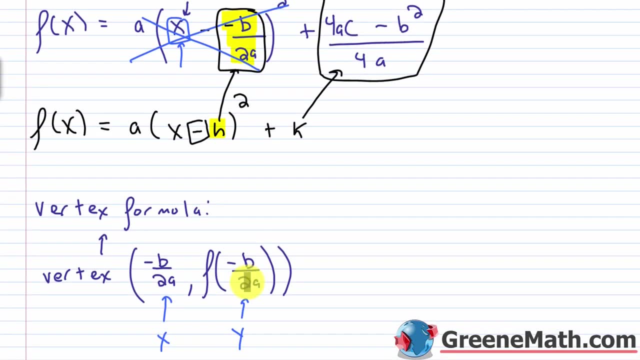 It would basically be zero, and I would be left with my value for k, which in this case is 4ac minus b, squared all over 4a. So that's why we put that there. It's just easier than writing 4ac minus b squared over 4a. 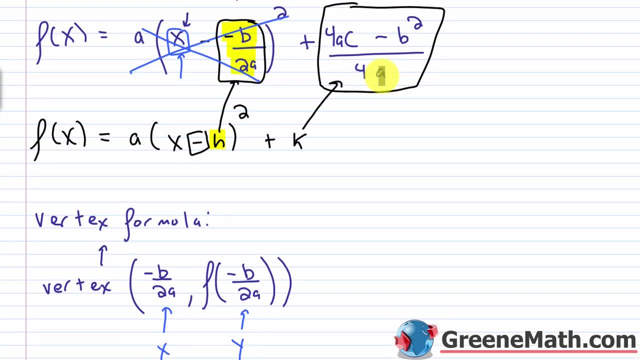 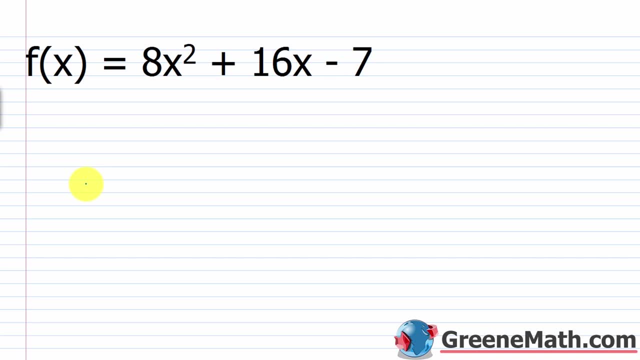 If you want to put that there, you can. It's the same answer either way. Okay, so let's try a few out. This is very, very simple. So we have: f of x is equal to 8x squared plus 16x minus 7.. 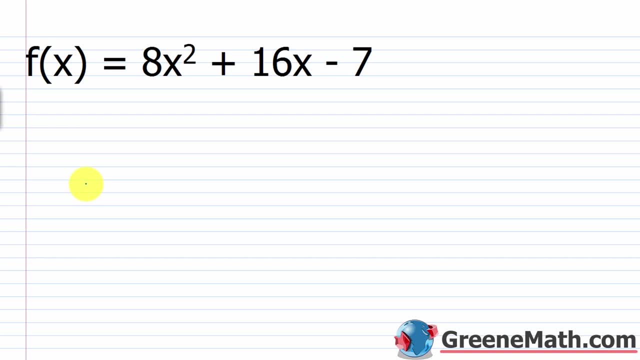 So we have a quadratic function in standard form. If you get one that's not in standard form, you need to put it in standard form, Okay, so if you see that trick question on the test, make sure it's in standard form. 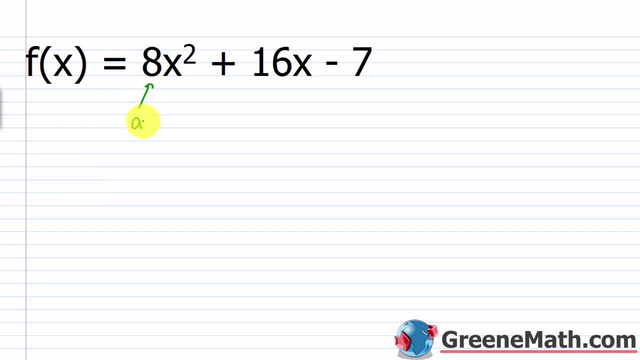 So what's my A? that's the coefficient for the squared variable. What's my b? That's the coefficient for the variable to the first power And for the formula I gave you. you don't need c, but just in case you want it. 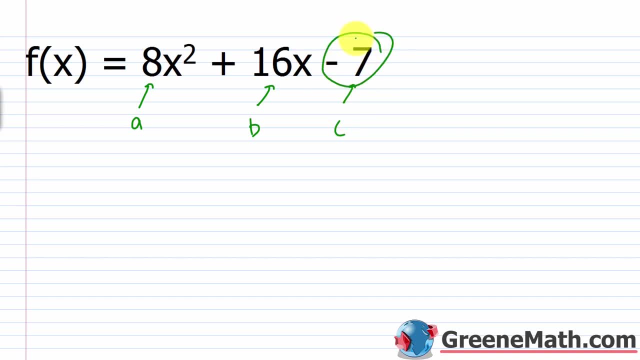 c is going to be negative 7.. That's the constant. So a is 8, b is 16, c is negative 7.. Okay, so I want to find the vertex. So the vertex occurs at negative b over 2a. 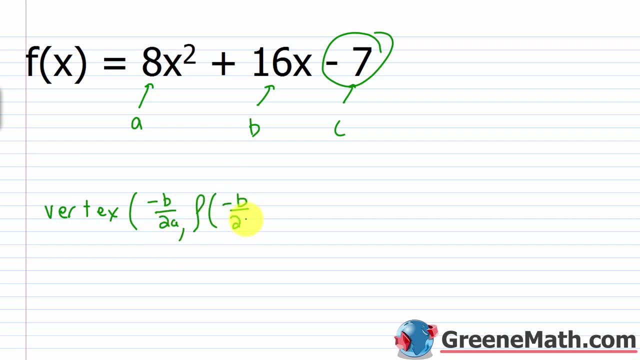 comma f of negative 7.. Okay, so I want to find the vertex at negative b over 2a. Okay so what's negative b? b here is 16.. So negative 16 over 2a a is 8, so 2 times 8 is 16.. 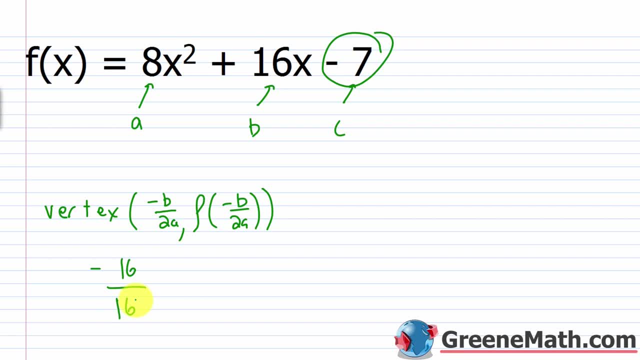 Negative 16 over 16 is negative 1.. So the vertex: the vertex occurs at negative 1, comma. Then what I want to do, I want f of negative b over 2a. We know negative b over 2a is negative 1.. 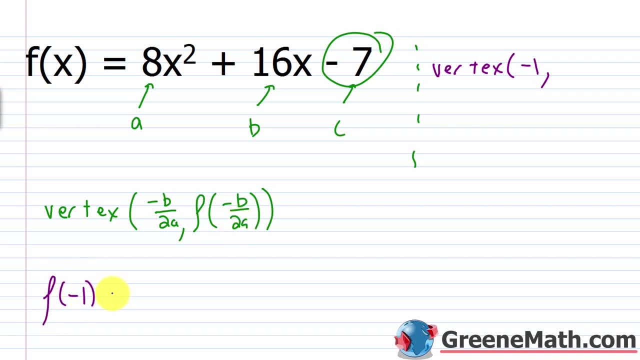 So we want f of negative 1. And this is equal to 8 times. you'd have negative 1 squared plus 16 times negative 1, and then minus 7.. So if we had negative 1 squared, that would be 1.. 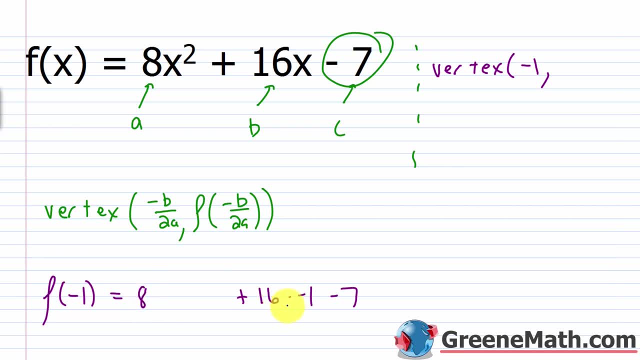 So this is basically 8 times 1, or 8.. And then if you had 16 times negative 1, that's negative 16. So this would be minus 16, and then minus 7.. So 8 minus 16 is negative 8.. 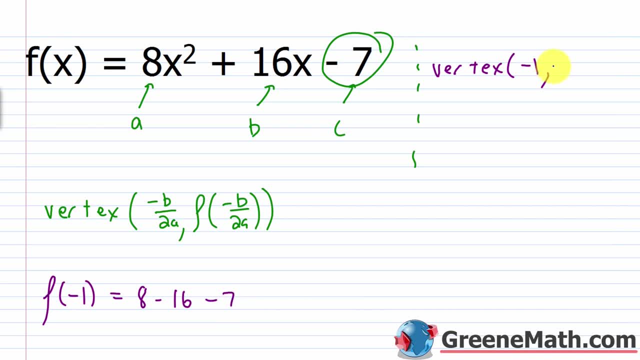 Then negative 8 minus 7 is negative 15.. So this would be negative 15 here. So f of negative 1 is negative 15.. So just that quickly we found our vertex. No messy completing the square, No long, lengthy process. 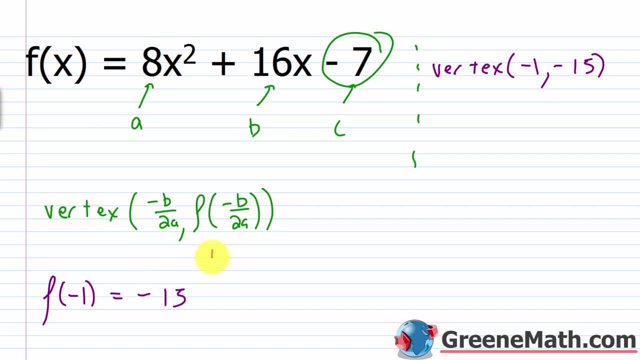 Pretty straightforward. So all you have to do is kind of write this down and understand how to find a, b and c, which is very, very simple, And you will have your vertex right away. So, once again, the vertex here is at the point negative 1, comma negative 15.. 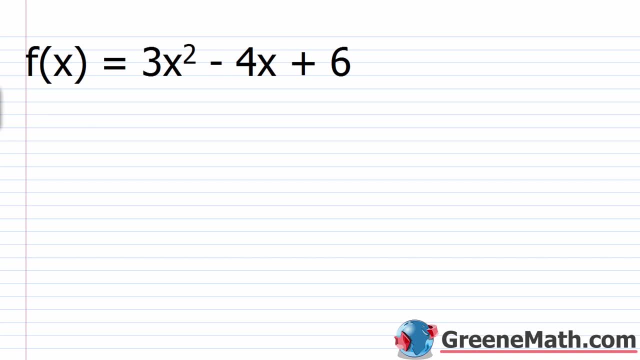 All right, let's try another one. So we have f of x equals 3x squared minus 4x plus 6.. So again the vertex formula. The vertex will occur at negative b over 2a, comma. f of negative b over 2a. 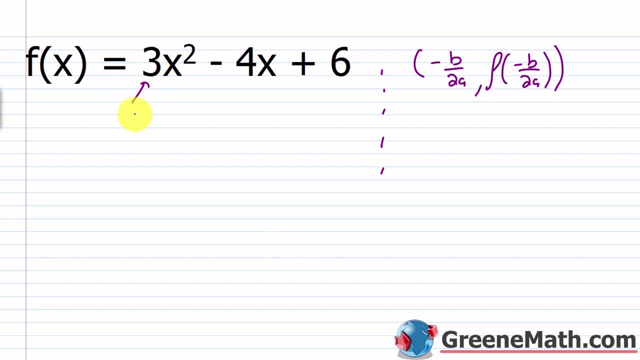 OK, so for negative b over 2a, this is a, this is b and this is c. So negative b, b is negative, 4.. So the negative of negative 4 is positive. 4 over 2a, a is 3.. 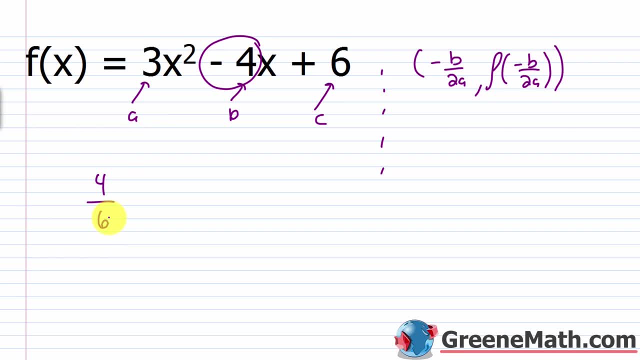 2 times 3 is 6.. So we'd have 4, 6.. We could reduce that to 2 thirds, So the vertex will occur. You'd have 2 thirds for the x location comma. Then you would have f of 2 thirds. 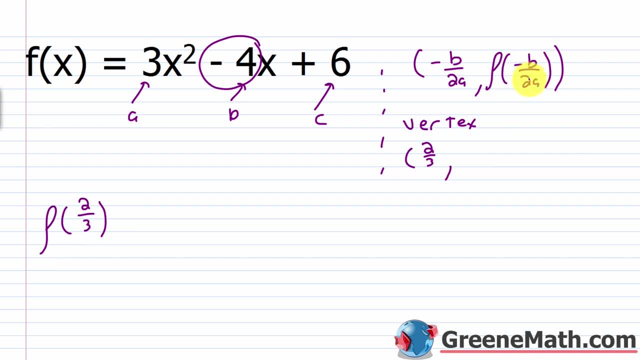 f of 2 thirds. right, It's f of negative b over 2a. We found that negative b over 2a was 2 thirds, So it's f of 2 thirds. So this would be equal to 3 times 2 thirds squared. 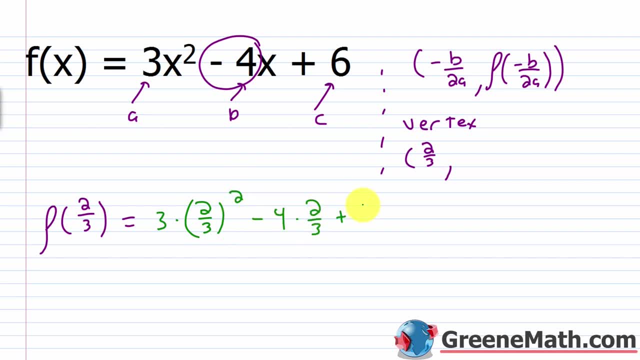 Minus 4 times 2 thirds plus 6.. If I square 2 thirds, I would get 4 ninths. So this would be 4 ninths And then 3 times 4 ninths. This would cancel with this and leave me with a 3 down here. 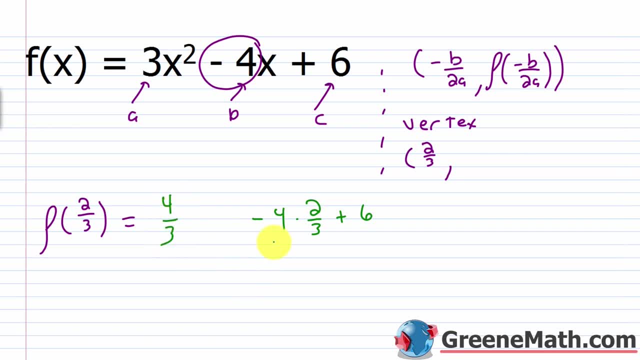 So this would be 4 thirds. So I'd have 4 thirds here, Then negative 4 times 2 thirds. You think about that as negative 8 thirds. So we'll say minus 8 thirds, Then you have plus 6.. 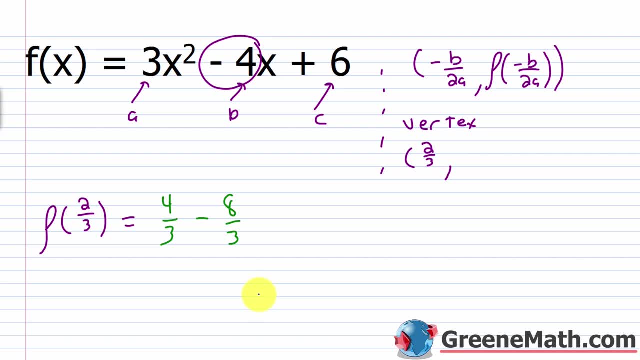 6. if I multiply by 3 over 3 to get a common denominator, That would be plus 18 thirds, And then I could say 4 minus 8 is negative 4. Negative 4 plus 18 is 14.. So this would end up being 14 thirds. 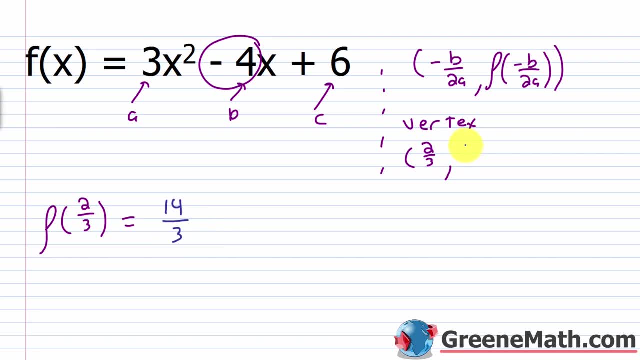 So f of 2 thirds equals 14 thirds, And that's going to be my location for y for that ordered pair. So the vertex occurs at the point 2 thirds, comma 14 thirds. All right, So now let's talk about the discriminant. 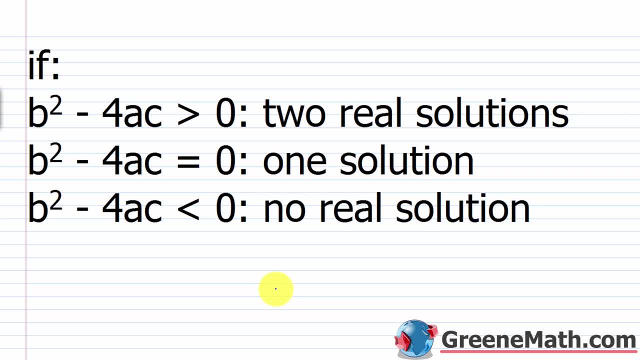 So you'll recall, when we solved quadratic equations we saw ax squared plus bx plus c equals 0. And we derived the quadratic formula. So if we want to solve something in this form, we can say that x is equal to negative, b plus or minus the square root of b squared minus 4ac, all over 2x. 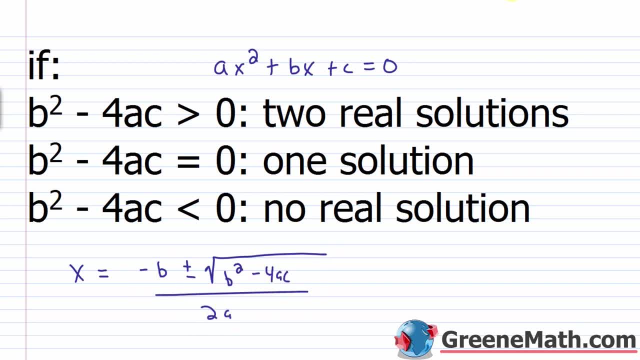 All right. So what we're going to focus on here is this part under the square root symbol. This is known as the discriminant. Now, the discriminant gives us information about the number of x-intercepts we're going to get, And we'll cover that in a second. 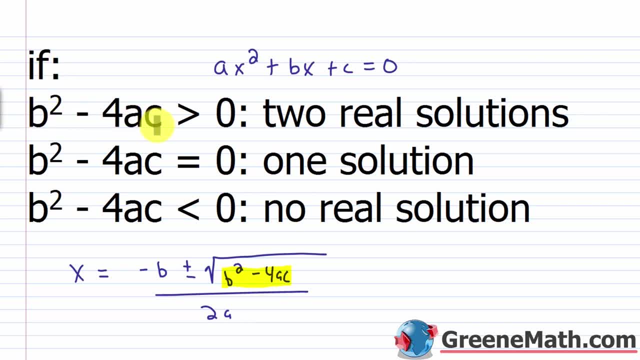 But for right now we just want to say: if b squared minus 4ac is greater than 0, we're going to have two real solutions And therefore you'll see in a second two x-intercepts If b squared minus 4ac is equal to 0,. 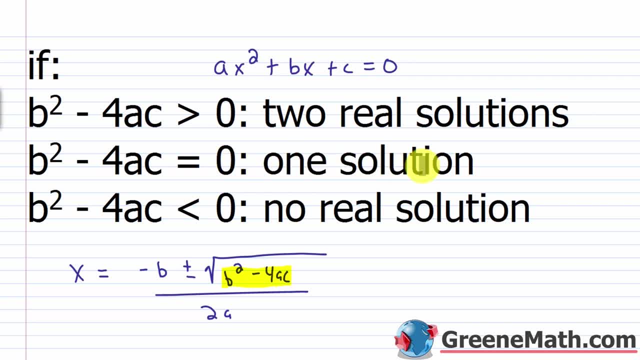 you're going to have one solution and therefore one x-intercept. You might say: well, why do you only have one solution here? If this guy was 0, the square root of 0 is 0.. So you have plus or minus 0.. 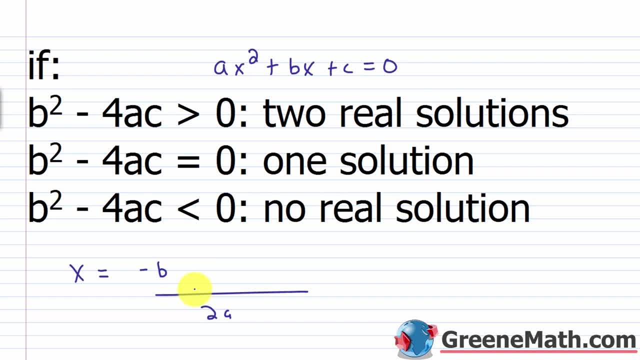 That's basically nothing right. You can get rid of that And you just have negative b over 2a. That's your solution. The last scenario is that b squared minus 4ac is less than 0.. So when we see this: 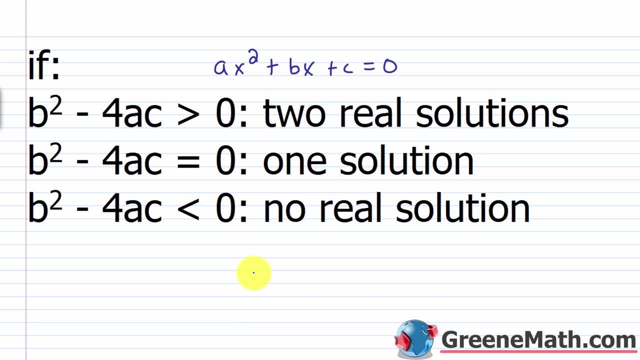 we don't have a real solution. Remember, we covered what to do in this case. You use complex numbers, right, We bring in our imaginary unit i, But when this occurs, we will not have an x-intercept. All right, 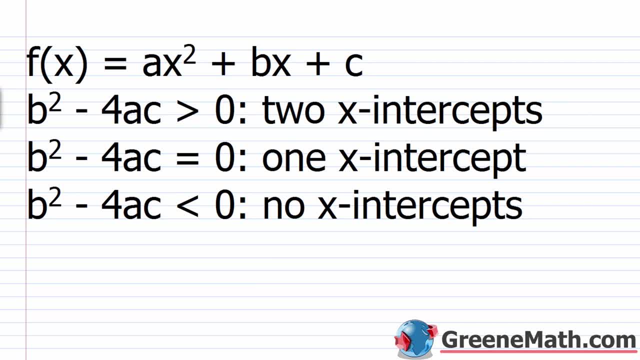 So here we have: f of x equals ax squared plus bx plus c. And if we allow f of x or y- OK, think about this as y for a minute- to be 0, what are we saying? Remember when we talked about linear equations? 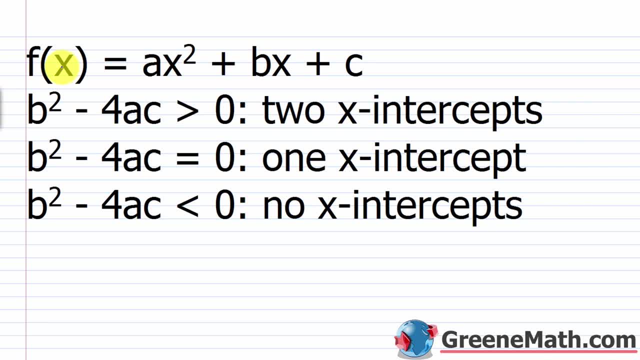 When y was 0 and we solved for x. we're refining the x-intercept right, Because it's the point where y is 0. So we are going to cross the x-axis. So if there are two solutions, as in b, squared minus 4ac is greater than 0,. 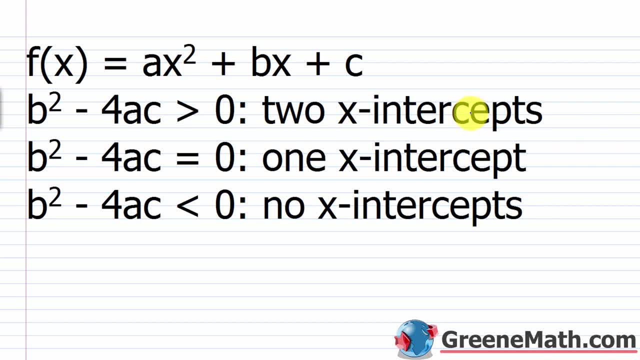 we're going to have two x-intercepts or two spots where that graph is going to cross the x-axis when y is equal to 0. Then, if b squared minus 4ac equals 0,, one x-intercept, And then if b squared minus 4ac is less than 0,. 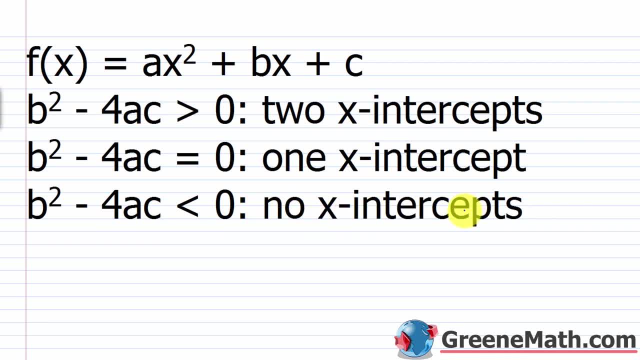 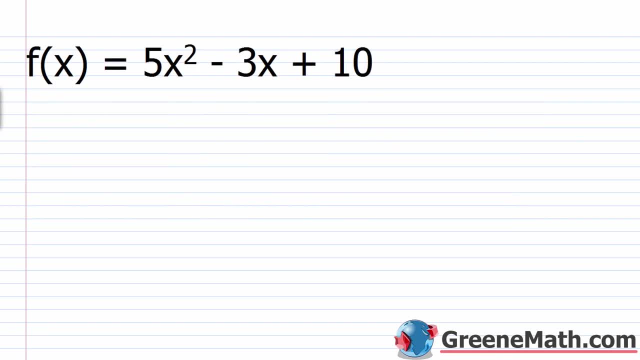 then no x-intercepts, right? So if you don't have a real solution, you will not find an x-intercept. So if we looked at this example, f of x equals 5x squared minus 3x plus 10,. 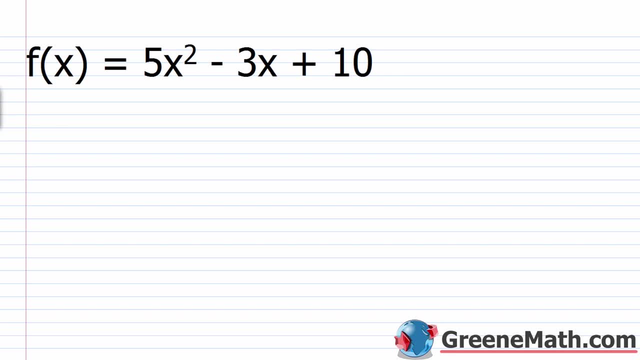 and we said how many x-intercepts will be here. Well again, you just look at your discriminant. So that's b squared minus 4ac, a is 5. b is negative, 3. c is 10.. 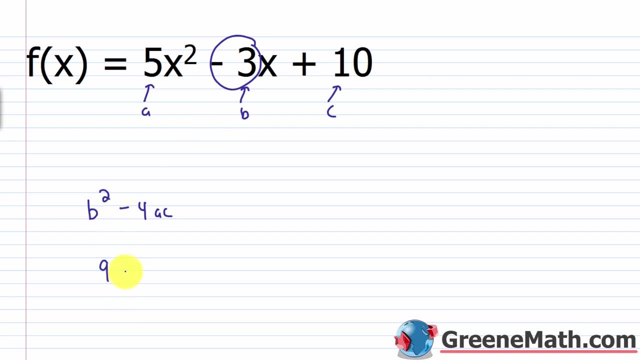 So what is b squared Negative? 3 squared is 9, minus 4 times a is 5, times c is 10.. So just looking at that, I know that this is going to be less than 0.. 4 times 5 is 20.. 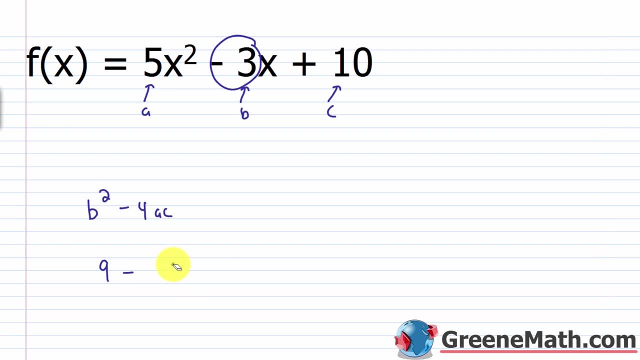 20 times 10 is 200. You would have 9 minus 200, which turns out to be negative 191, and negative 191 is less than 0. So again, if the part that's underneath the square root symbol is negative, 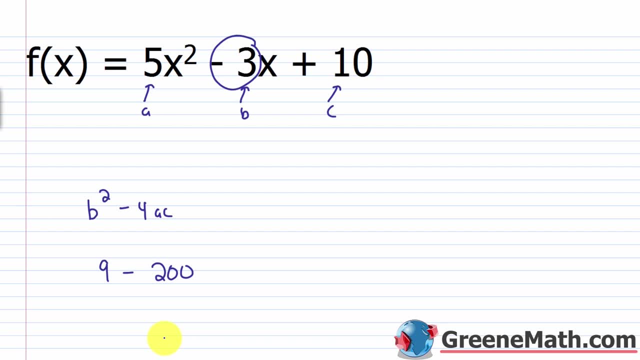 you know you're not going to have a real solution. So when this is less than 0, there's no real solution, and so there's no x-intercepts, So 0x-intercepts All right. If we looked at another one. 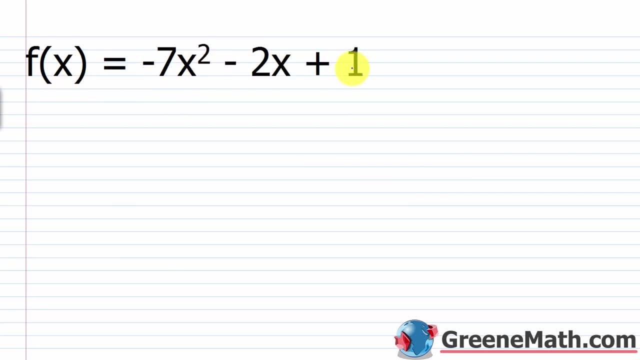 we have f of x equals negative 7x squared minus 2x plus 1. So again we're looking to see how many x-intercepts we have. So this is my a negative 7.. This is my b, negative, 2.. 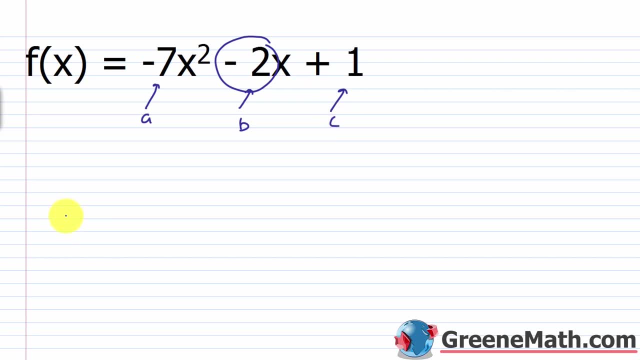 And this is my c: 1.. So the discriminant is b squared, so negative 2 squared, that's 4, minus 4 times a. a is negative 7, times c, c is 1.. So you might as well say this: is plus negative 4. 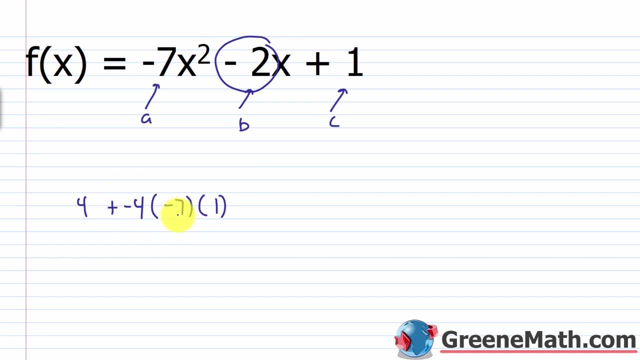 to make it easy: Negative 4 times negative, 7 is positive 28.. 28 times 1 is still 28.. So this is 28.. And without even doing the addition, we know this is positive. so we know that there are two real solutions. 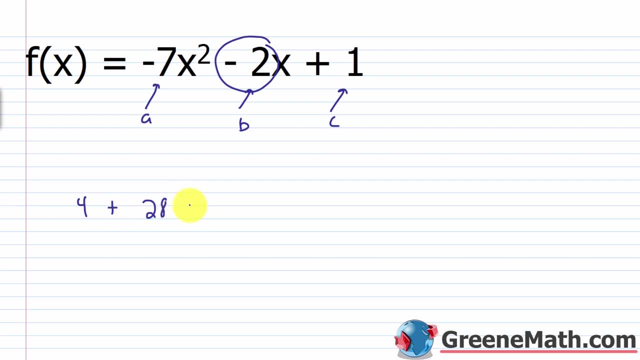 or 2x-intercepts. 4 plus 28 will give me 32.. So 2x-intercepts, All right. So another thing to consider if we're graphing a quadratic function, if a is greater than 0,. 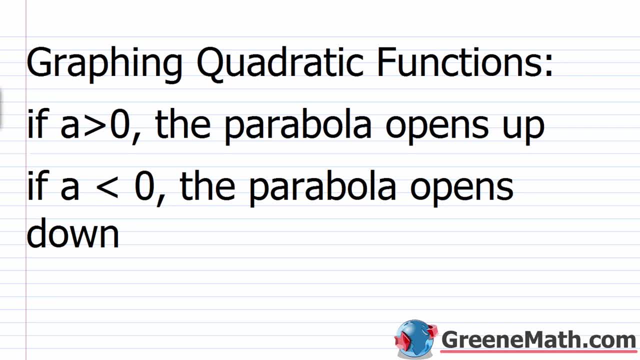 the parabola is going to open up. If a is less than 0, the parabola is going to open down. So a again is the coefficient of the squared variable. Okay, The coefficient of the squared variable. So if that's positive, 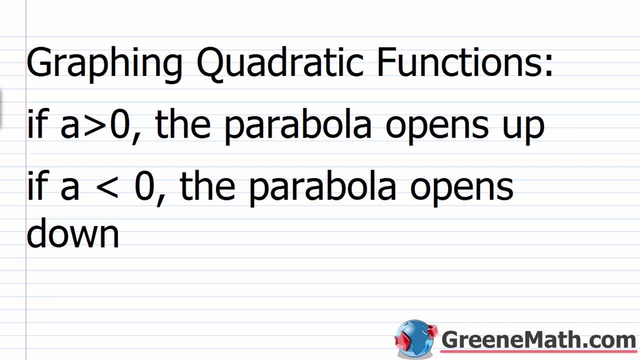 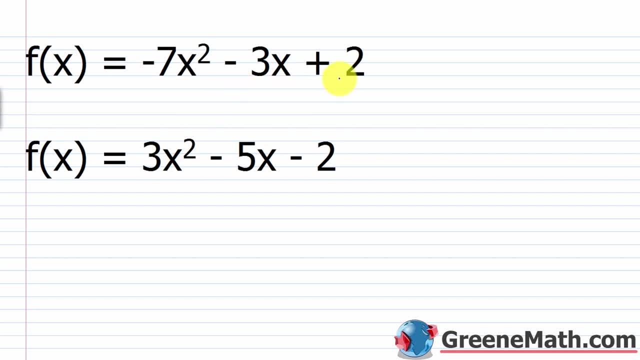 you're going to have a u-shape. If it's negative, you're going to have an upside-down u-shape. So two examples here We have: f of x equals negative, 7x squared minus 3x plus 2.. 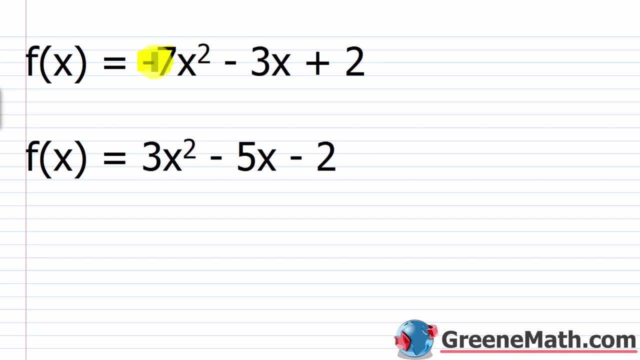 In this case, the negative 7 here tells me that this guy is going to open down. Right, It's going to open down. For this one, f of x equals 3x squared minus 5x minus 2,. the positive 3 tells me this guy is going to open up. 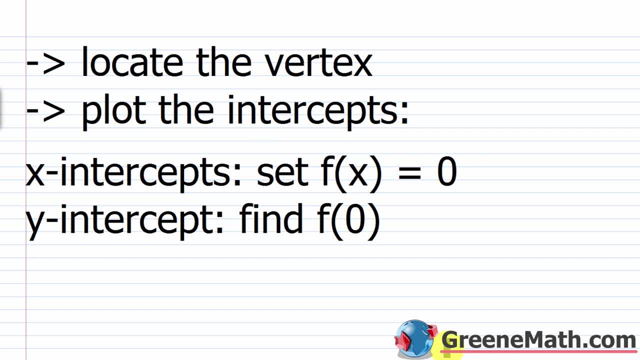 All right. So if you wanted to graph a quadratic function, if your teacher made you do it, just as an exercise to see if you could, the first thing you would do is determine if the graph opens up or down. Again, look at the value for a. 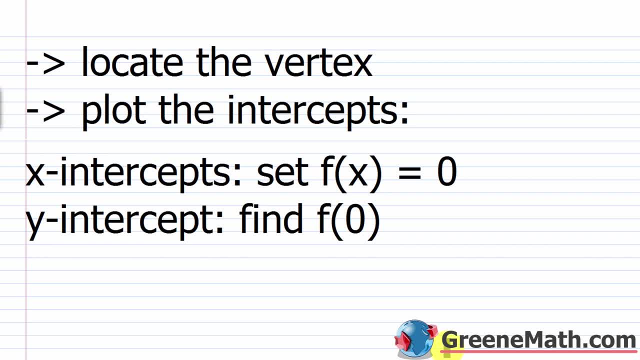 Is it positive, It opens up. Is it negative, It opens down. Then you want to locate the vertex. We have the vertex formula for that. That's pretty easy. So you want to plot the x-intercepts, if you have them. 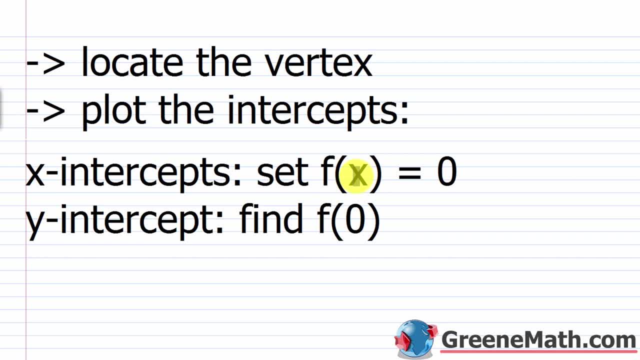 Again, f of x or y will be equal to 0.. So you're solving: ax squared plus bx plus c equals 0. What we've been solving forever, right? We can use the quadratic formula for that And then for the y-intercept. 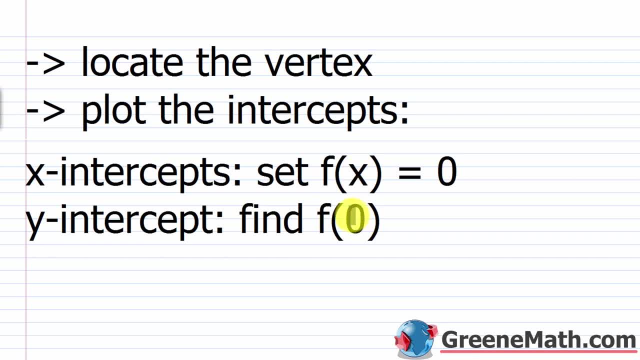 you want to find f of 0. Okay, Remember, if I am plugging in for x in function notation, I just put what I want to plug in right there. So f of 0 means I'm going to plug in a 0 for x. 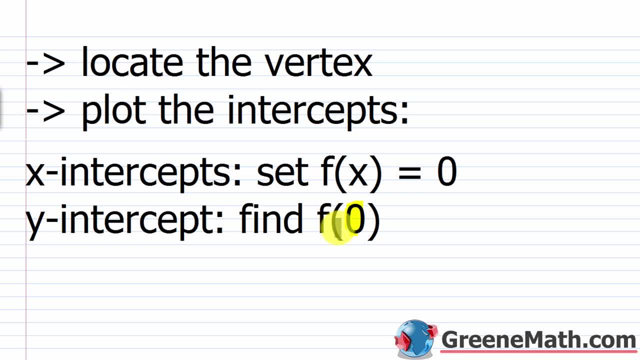 And again, we know this from graphing linear equations: If I plug a 0 in for x, I'm finding the point where x is 0 and I'm crossing the y-axis. Okay, So you give me my y-intercept. 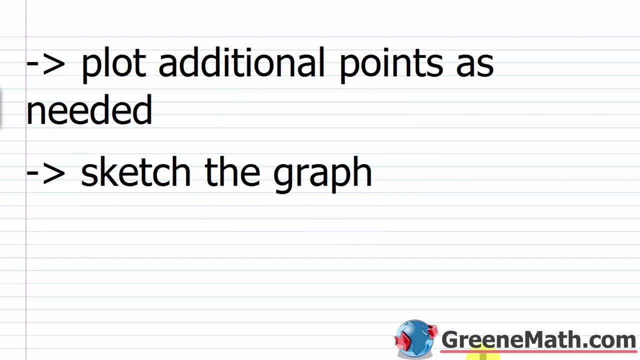 All right, Then I want to plot additional points as needed. To graph a parabola, you only need three points, But again, you're not graphing a line, So the shape isn't always 100% clear. Again, that's why we use these graphing calculators. 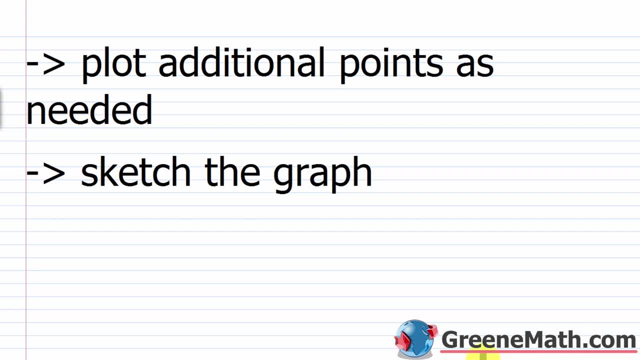 and software to kind of do this for us so that it's accurate. Then, lastly, you will sketch the graph. Okay, So let's give one of these a shot. I'm just going to do one And then, if you want to do some additional practice on that, 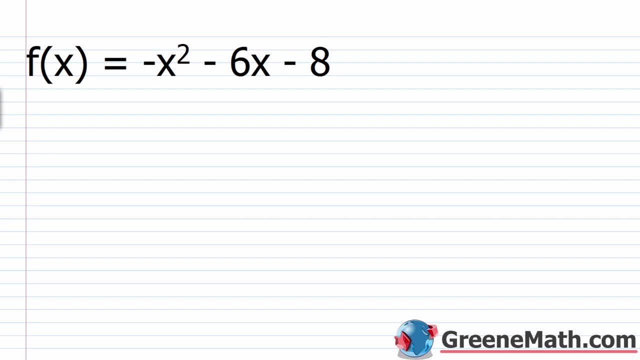 that's fine. But again, I'm just going to tell you, as you move out of Algebra 2, you get into trigonometry and calculus and college algebra. most of the time you're not going to hand draw things, You're going to be using your graphing calculator. 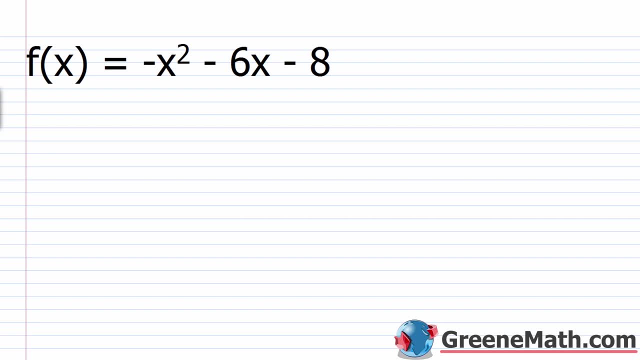 or some type of graphing software, All right. So the first thing is this guy right here: f of x equals negative x squared minus 6x minus 8.. This is negative here, So I know it's going to open down. 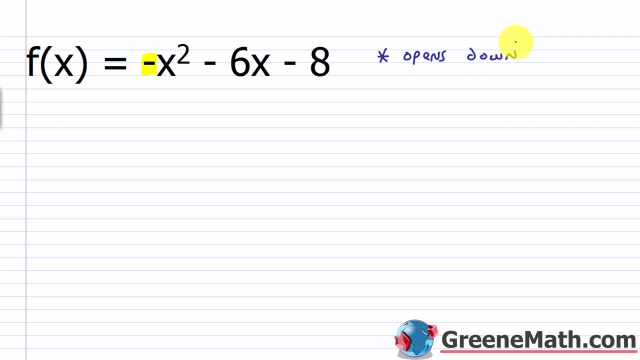 So opens down. So I know that It's going to have this shape right here. All right, So the next piece of information: what is the vertex? So the vertex? the vertex will occur where Negative b over 2a. 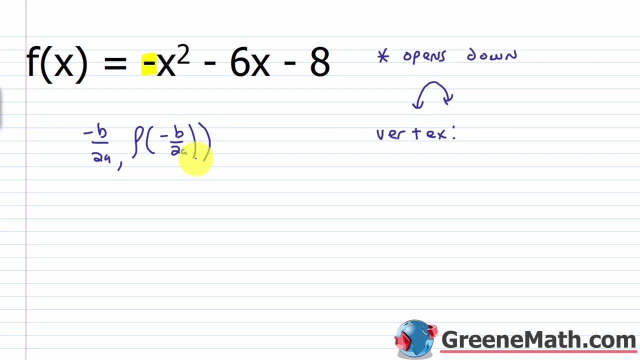 f of negative b over 2a. And what is a and b? So this is a That's negative 1.. And b is negative 6.. So the negative of negative 6 is 6 over 2 times negative 1,. 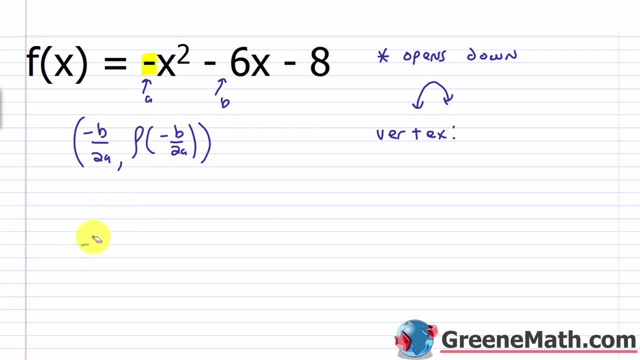 which is negative 2.. So 6 over negative 2 is negative 3. So the vertex will occur at negative 3 comma. Now I want to plug a negative 3 in for x, So I'd have f of negative 3.. 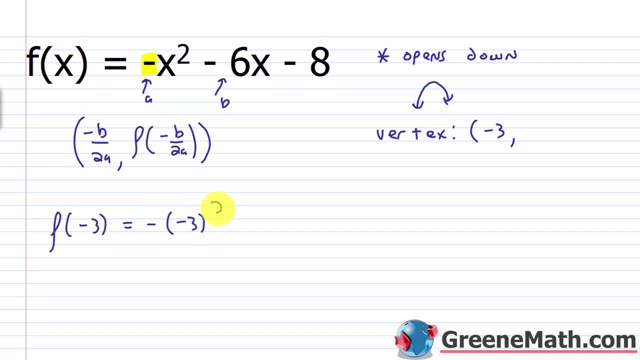 This would equal negative and then negative 3 squared minus 6, times negative 3, then minus 8.. Let's erase this. So negative 3 squared is 9.. So I'd have the negative of 9, just negative 9.. 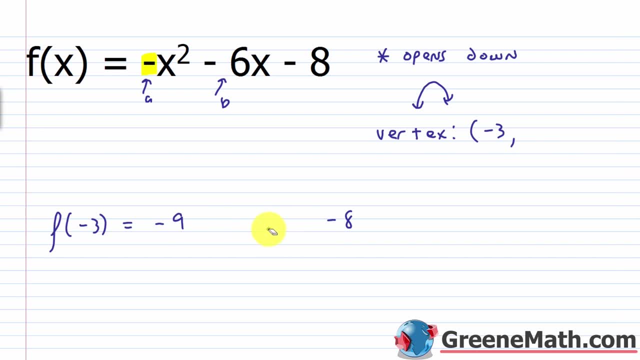 And then negative 6 times negative, 3 is positive 18. So this would be plus 18.. And then it would be minus 8.. So minus 8.. So negative 9 plus 18 is going to give me 9.. 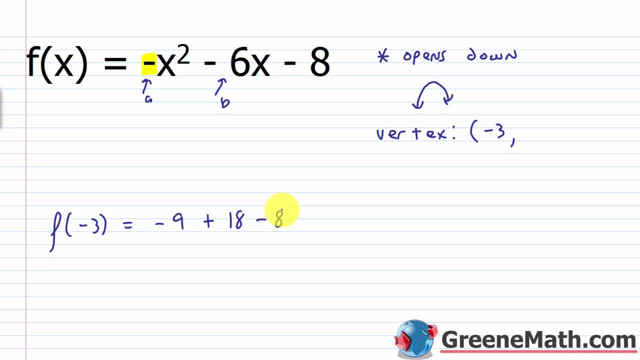 9 minus 8 is 1.. So the vertex will occur at negative 3 comma 1.. Okay, So now we want to figure out what our x-intercepts are. So we would set this equal to 0.. So we would say this is 0. 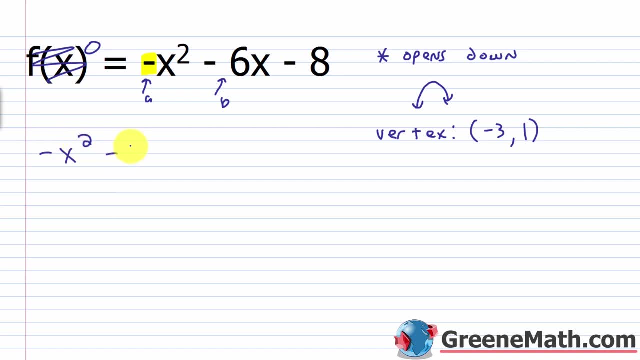 And I would just say, let's just solve negative x squared minus 6x minus 8 equals 0.. Again, I can use my quadratic formula for that: x is equal to negative b, b is negative 6. So the negative of negative 6 is 6.. 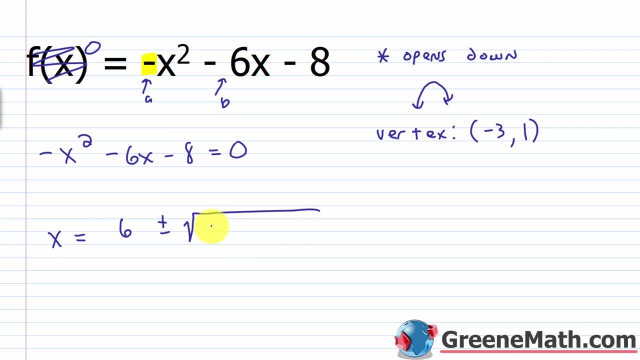 Plus or minus the square root of b squared Negative 6 squared is 36.. Minus 4 times a, a is negative 1.. Times c: c is negative 8.. This is all over 2a a is negative 1.. 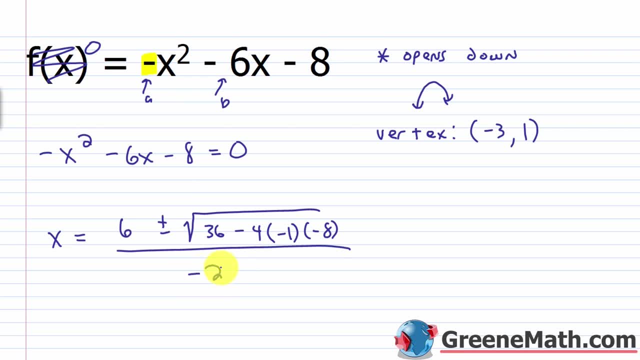 So 2 times negative 1 is negative 2.. So I think about this as plus negative 4 to make it easy Negative. 4 times negative 1 is 4.. 4 times negative 8 is negative 32.. 36 minus 32 is 4.. 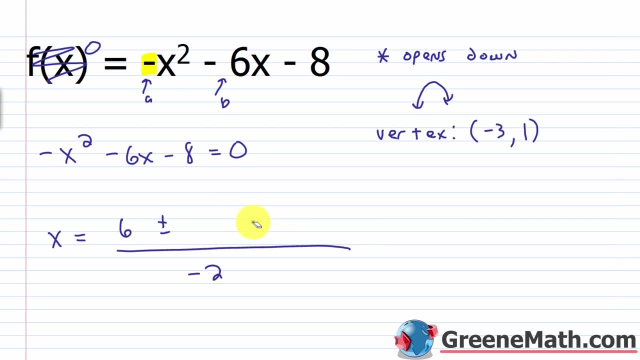 So you'd be taking the square root of 4, which is 2.. So your two scenarios here is: 6 plus 2 is 8.. 8 over negative 2 is negative 4.. And then your other scenario is: 6 minus 2 is 4.. 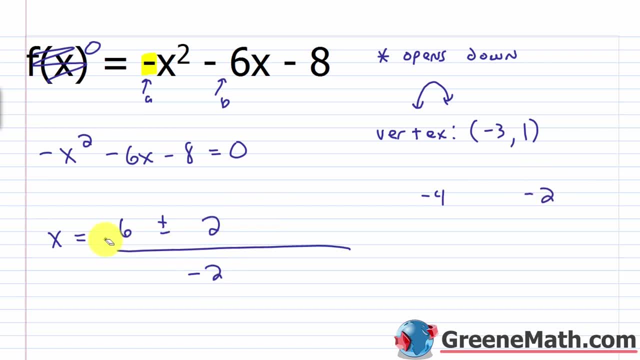 4 over negative 2 is negative 2.. So those are x values, But remember the y value is going to be 0 in each case. So we would say that our x-intercepts will occur at negative 4 comma 0. 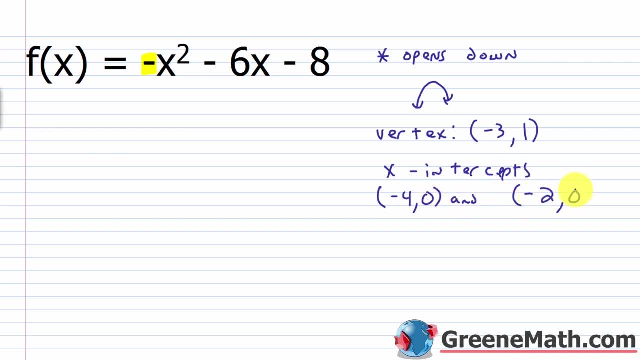 and negative 2 comma 0.. Now, where's our y-intercept going to occur To find that we want f of 0. I want to plug in a 0 for x. So if this was 0 and this was 0,. 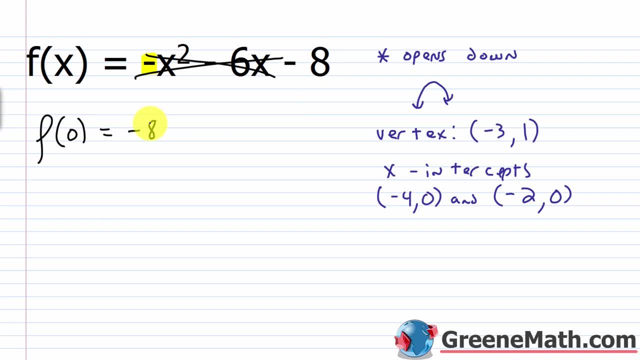 they'd basically be gone. I'd just have negative 8 there. So f of 0 is negative 8.. So we would have an x value of 0 and a y value of negative 8.. This is your y-intercept. 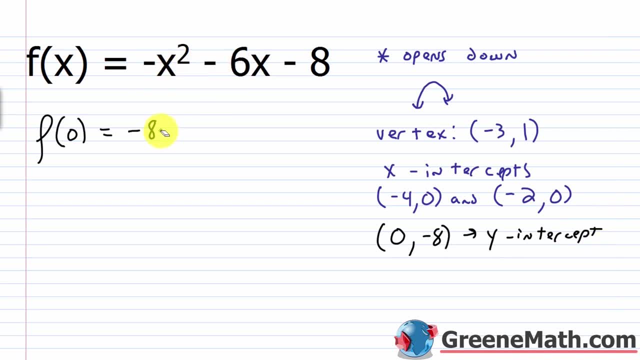 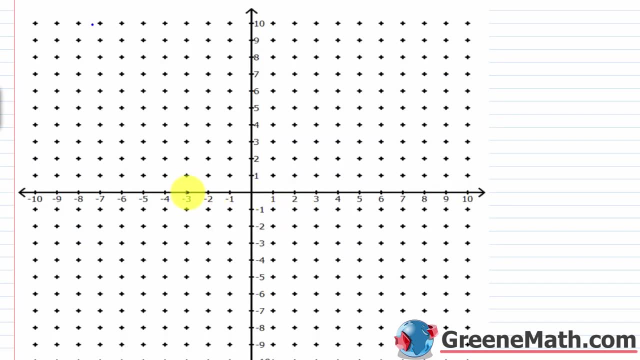 Now we might need additional points. Let's just go down to the graph and see what we're looking like. Let's start with the vertex. It's at negative 3 comma 1.. So 3 units to the left comma 1,. 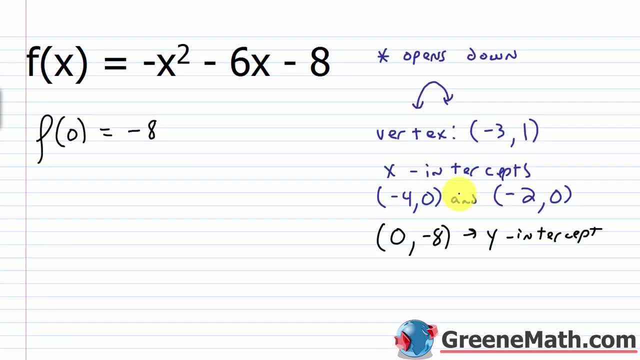 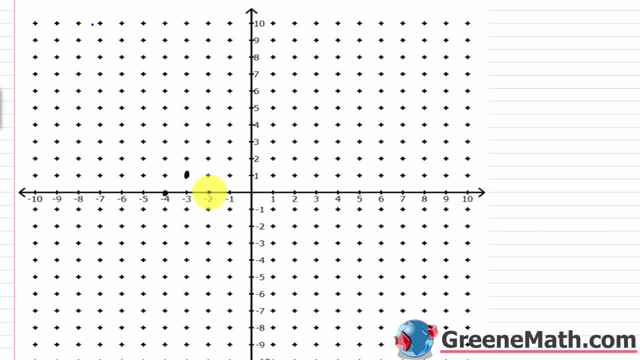 one unit up. And then the next point we want are x-intercepts. We have negative 4 comma 0 and negative 2 comma 0. So negative 4 comma 0 and negative 2 comma 0. So at this point 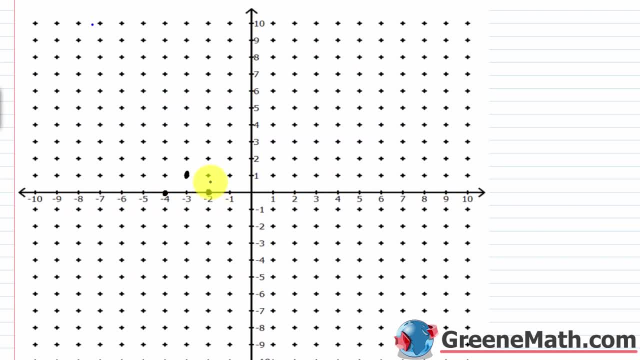 you have three points. You could sketch a parabola So you could start there. But the problem is you really don't get a good representation of where this thing is going to go, the angle and whatnot. So that's why you try to get some additional points. 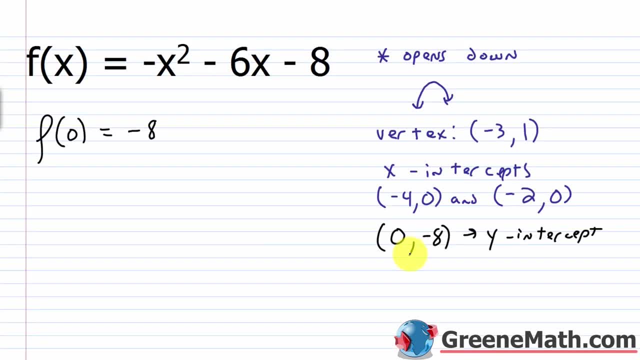 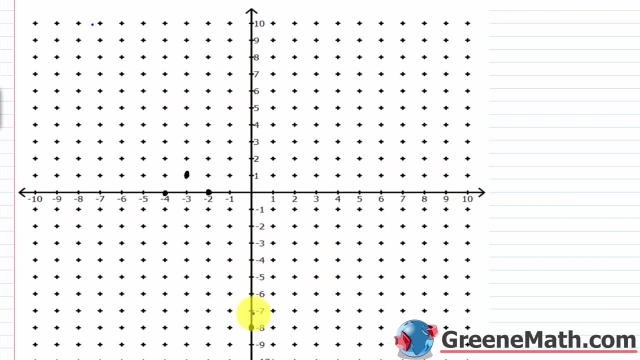 so you get more information. I know my y-intercept occurs at 0 comma, negative 8.. So 0 for the x location, negative 8 for the y location, And then we can get one additional point going. Let's figure out where x would be. 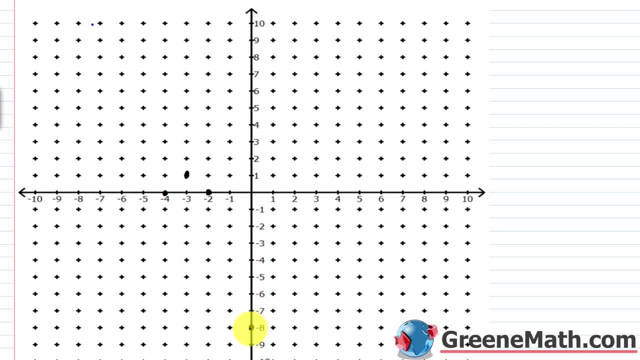 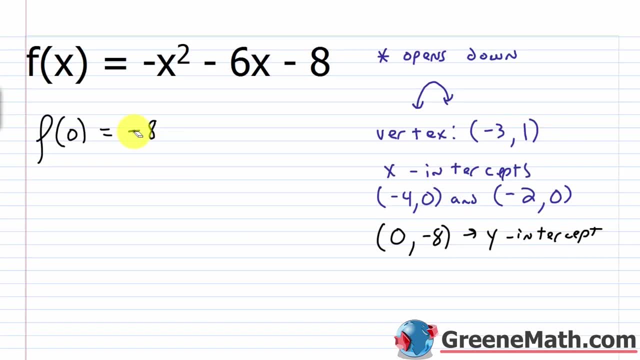 if y was negative 8.. So we know there's one place here at 0 comma negative 8, but what's the other place? So let's go and let's plug in a negative 8 for y or for f of x. 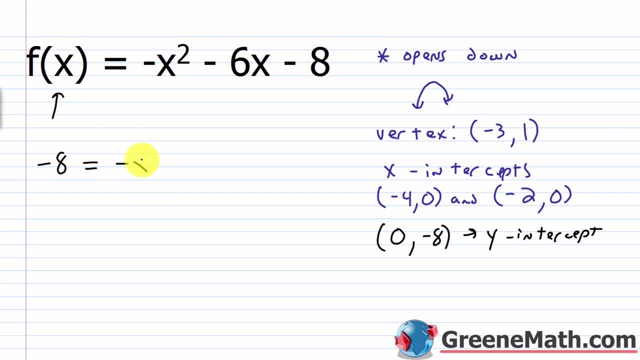 however you want to think about that. So negative 8 equals negative x squared minus 6x minus 8.. So I would add 8 to each side of the equation. This is gone. this is gone. So you have: negative x squared minus 6x is equal to 0.. 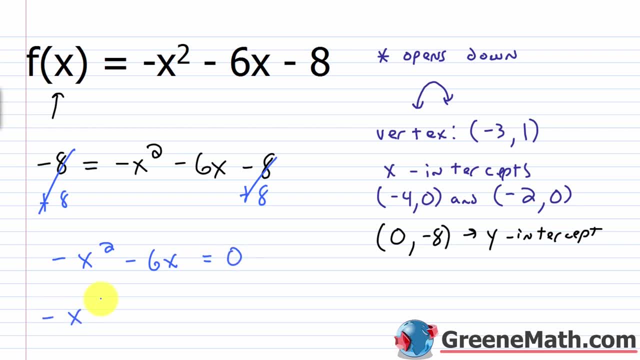 I could factor a negative x out there, So negative x, and then times the quantity, You would have an x plus 6 inside and this equals 0. So one solution is that x equals 0.. So we already have that with the y-intercept. 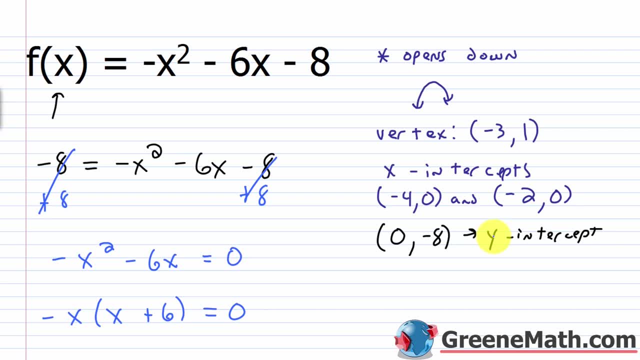 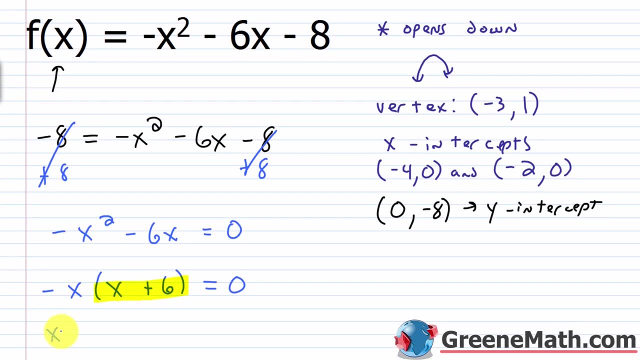 x is 0, y is negative 8.. We've got that. The other solution would come from this factor right here. If x plus 6 was equal to 0, if x plus 6 is equal to 0, subtract 6 away from each side of the equation. 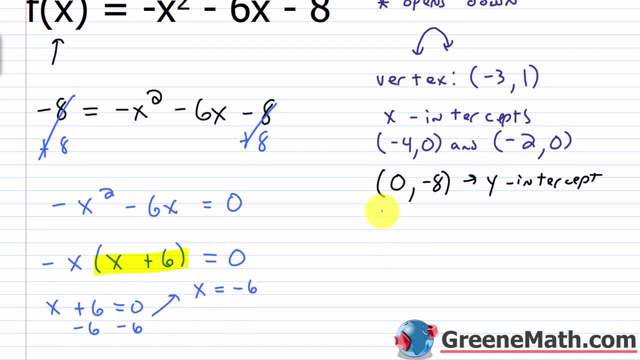 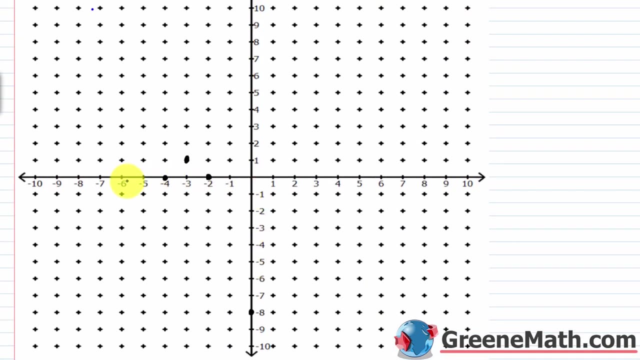 you say that x is equal to negative 6.. So an additional point would occur when x is negative 6 and y is negative 8.. This is an additional point. So negative 6, comma 8.. So that's going to be right there. 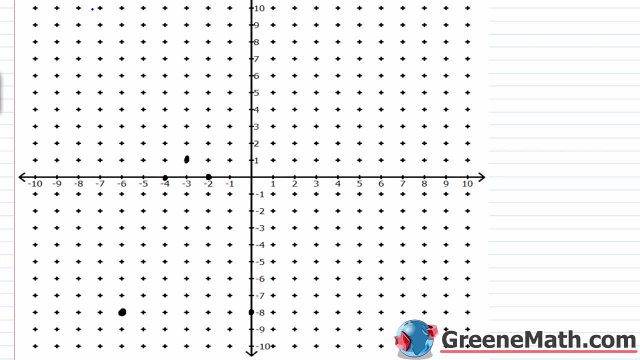 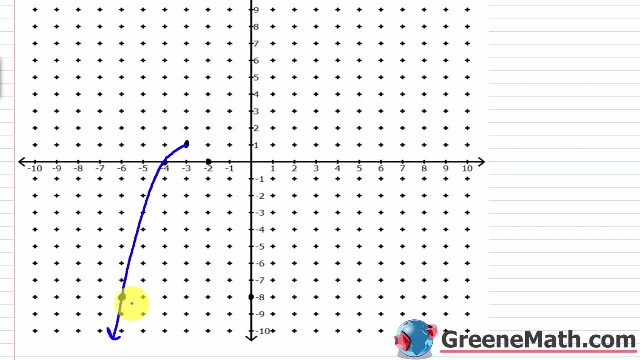 All right, So let's go ahead and attempt to graph this guy Again. I'm not a good drawer, but I'll do my best, So okay. So, not the best drawing in the world, I realize that, But if you wanted to see an accurate representation, 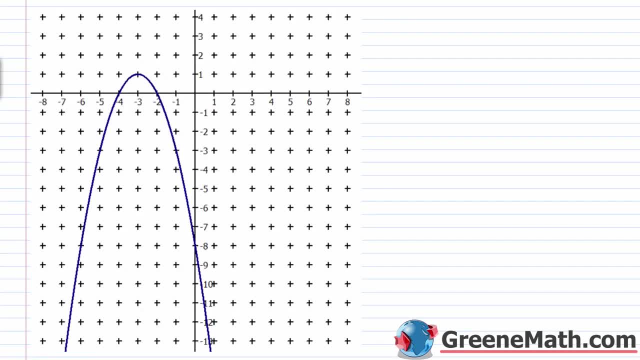 of what this looks like. we can look at a computer-drawn graph, for f of x equals negative x squared minus 6x minus 8.. Now the scale is a little bit different. My y-axis didn't go that far down. 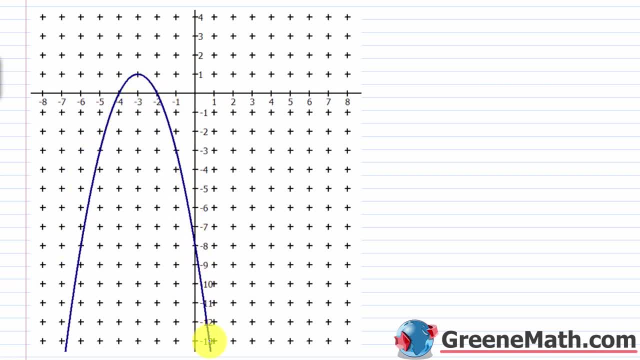 But again, you can see how perfectly drawn this is. And that's what you're going to get when you graph these things with some software, a graphing calculator, your computer, maybe some app on your phone. whatever you have, That's much preferable to hand drawing. 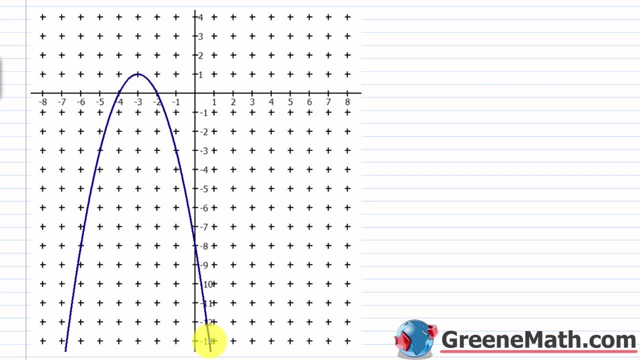 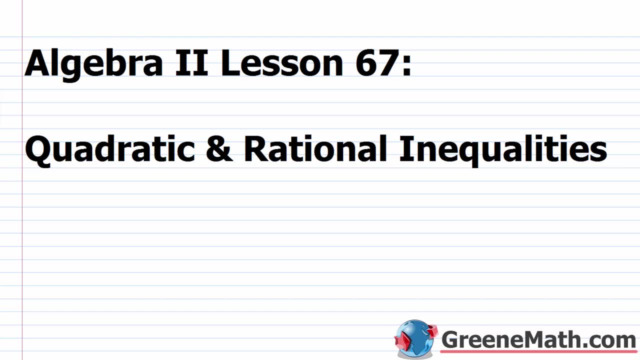 But again, if you need to hand draw it, at least you know the steps. Hello and welcome to Algebra 2, Lesson 67.. In this lesson we're going to learn about quadratic and rational inequalities. So we're going to start out by talking about 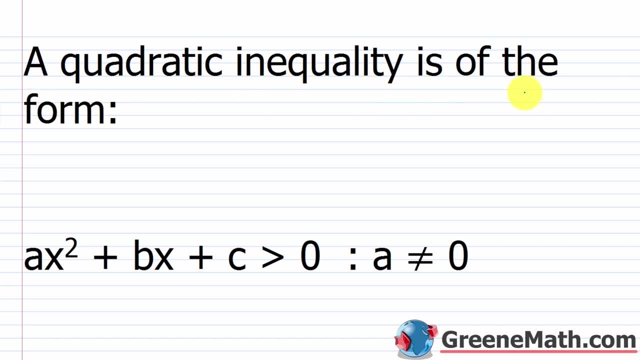 quadratic inequalities. And a quadratic inequality is of the form You'll see: ax squared plus bx plus c is greater than 0. And of course we have the restriction that a is not equal to 0. But other than that, a, b and c can be any real number that you choose. 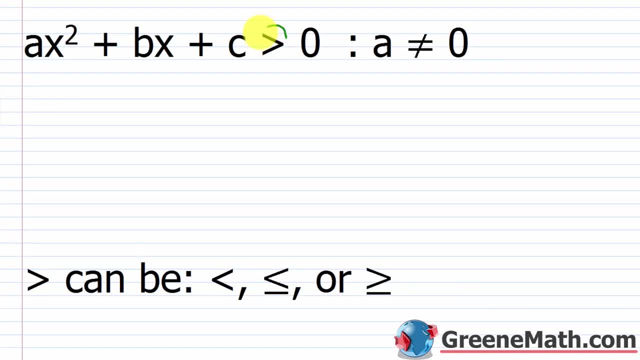 Of course, when we see something generically, we have to choose something to go there. So here we have a greater than, But of course the greater than can be a less than, a less than or equal to, or a greater than or equal to. 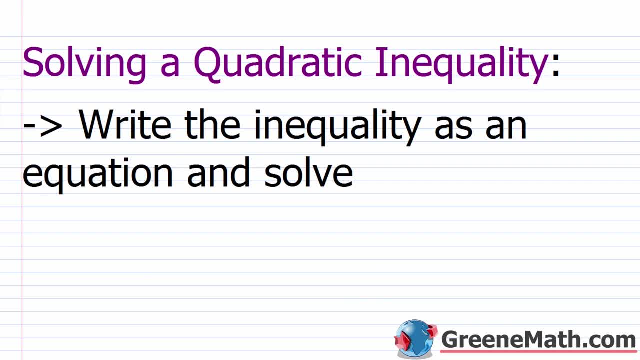 So, before we jump into how to solve a quadratic inequality, I just want you to think back for a moment to when we solved a linear inequality in two variables. The very first thing we did was to replace the inequality symbol with an equal symbol. That gave us a linear equation in two variables. 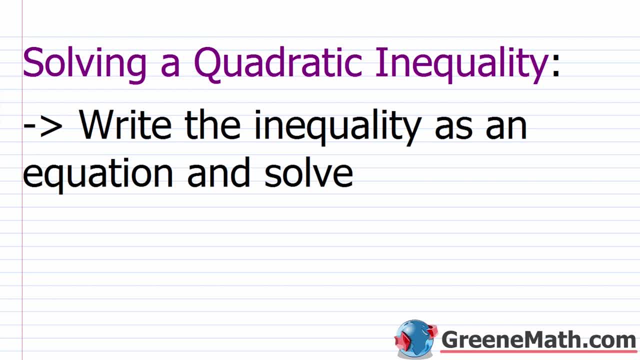 And we were able to graph the resulting line. Now that line had a special name. It was called the boundary line. And what's important about the boundary line is it separates the coordinate plane into two regions. One region would be the solution region. 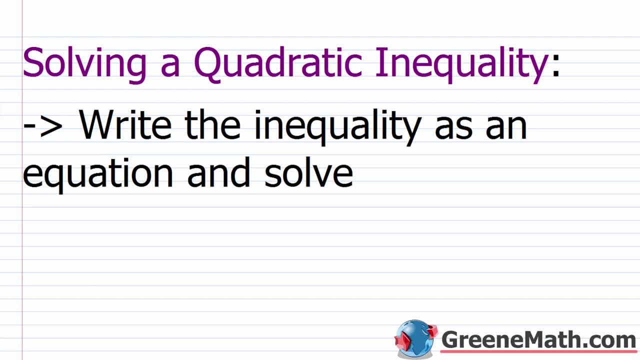 So everything in that region satisfied the inequality. The other side of the boundary line would be the non-solution region, So everything on that side would not satisfy the inequality. So from understanding that we come up with this idea of a test point, 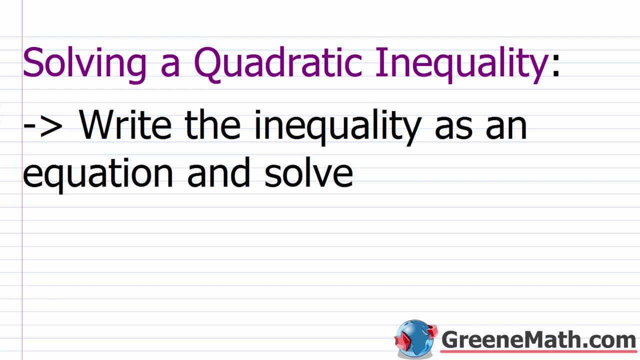 I can figure out where the solution region is by grabbing a point on either side of that boundary line, plugging into the original inequality and seeing if I get a true statement. If I get a true statement, that means my test point is in the solution region. 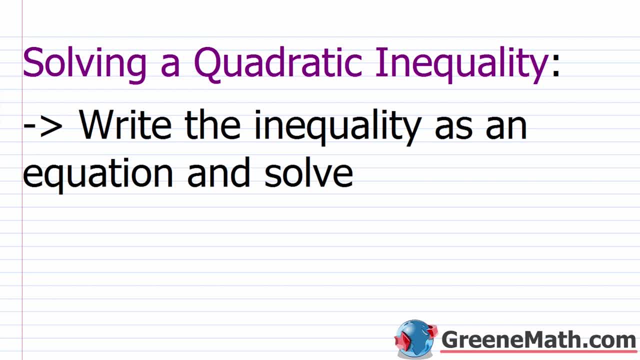 If I get a false statement, that means my test point is not in the solution region And the other region on the other side of that boundary line is going to be the solution region. Now another important thing to kind of note here before we move into this process. 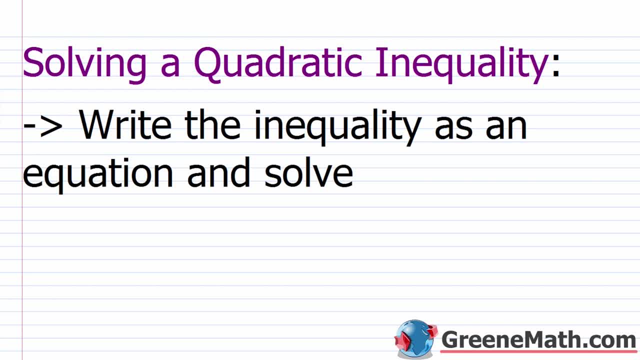 the boundary line, remember, was part of your solution if you had a non-strict inequality and it was not part of your solution if you had a strict inequality. You're going to see that thinking about that process just for a minute is going to bring back some things. 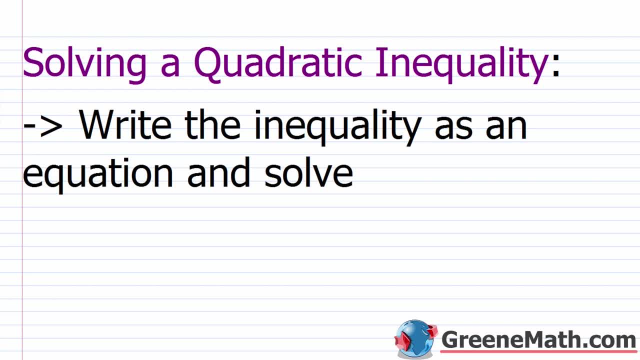 that are going to help you get through this here. Alright, so when we're solving a quadratic inequality, the very first thing you're going to do is you're going to write the inequality as an equation and you're going to solve that equation. 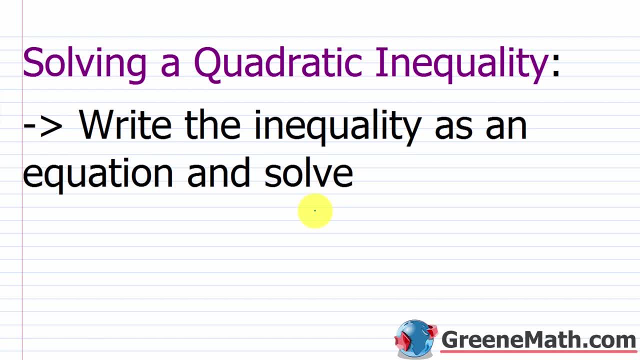 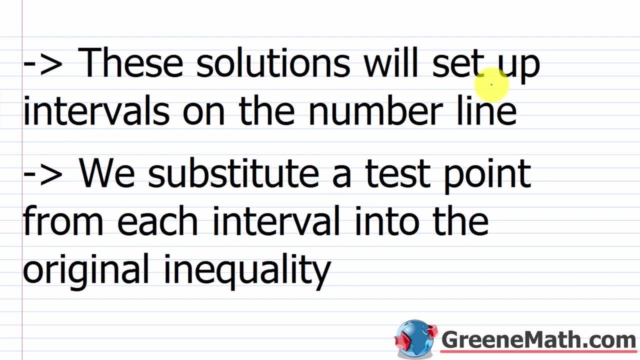 So this is going to give you a quadratic equation and you can just use the quadratic formula or, in some easier examples, you'll be able to factor this guy and just use your zero product property. So once you've obtained the solutions from your quadratic equation, 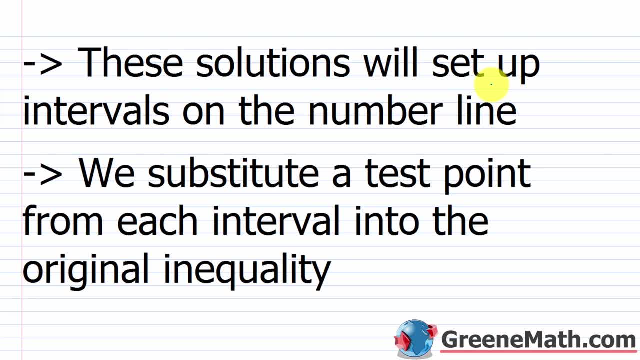 these solutions will be used on a number line, So this is going to be an old-fashioned number line, one you learned back in pre-algebra, and essentially this is going to tell us what the boundary points are, or the end points. 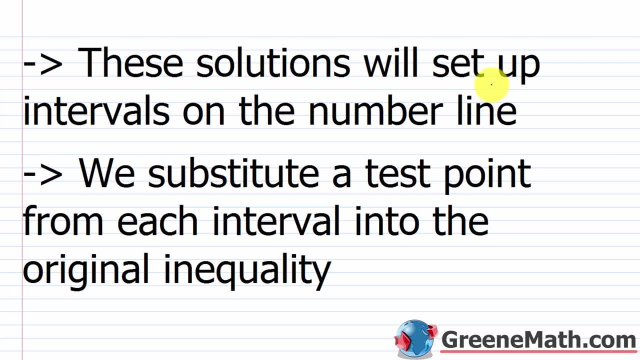 So these will be the points that separate the solution region from the non-solution region. So, essentially, these solutions will set up intervals on the number line And you'll see this in a minute when we get to an example. Essentially in each interval, 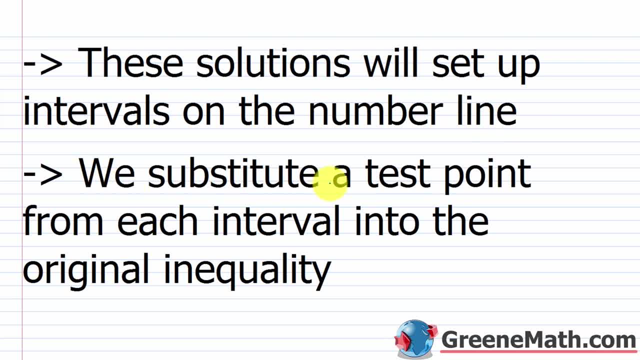 you can grab a test point, okay. So we substitute a test point from each interval into the original inequality. So obviously, if the test point is successful, meaning it satisfies the inequality, that interval is part of the solution set. If it fails, 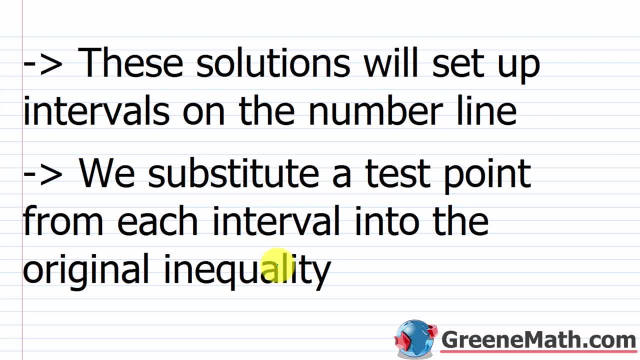 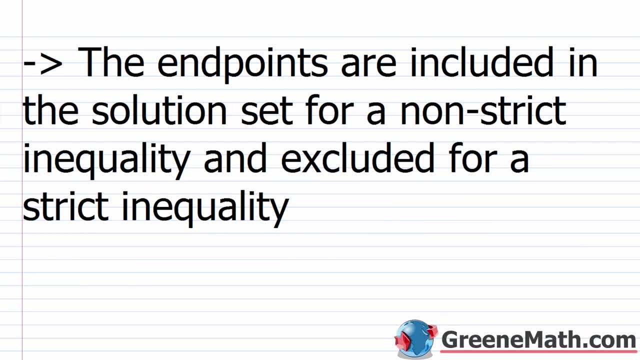 if it produces a false result, then that interval is not part of the solution set. All right now. lastly, the end points or the boundary points, however you want to call it. they are included in the solution set for a non-strict. 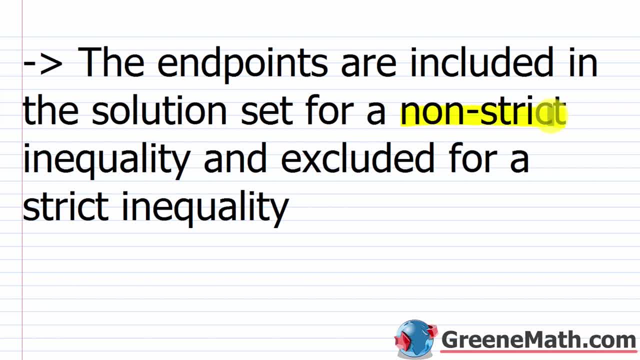 a non-strict. so you have a greater than or equal to, or a less than or equal to inequality and excluded for a strict inequality. So if you have strictly less than or strictly greater than, they're going to be excluded from the solution. 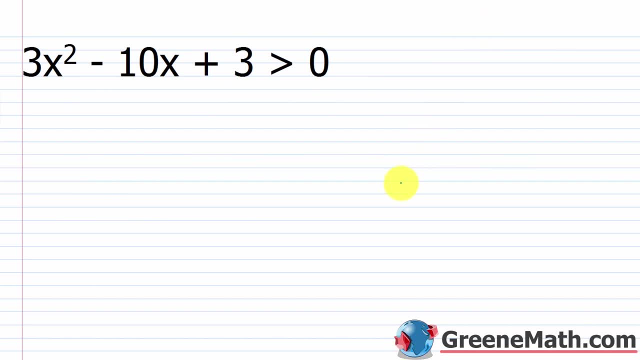 Okay. so now let's jump in and just look at a problem. Once we kind of get going on these, you'll see that they're very, very easy to solve. So we have 3x squared minus 10x plus 3. 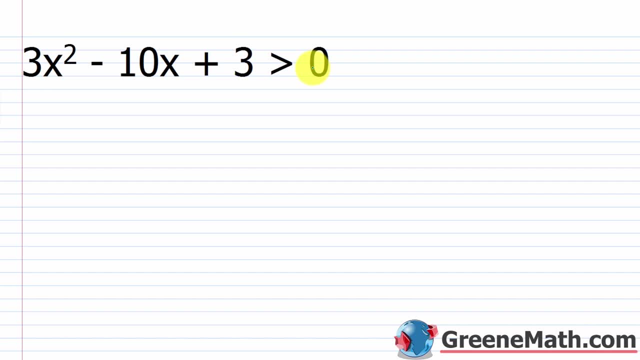 is greater than 0.. So the very first thing I want to do is I want to make this into an equation. So 3x squared minus 10x plus 3 is equal to 0, okay, So I know that this is a quadratic equation. 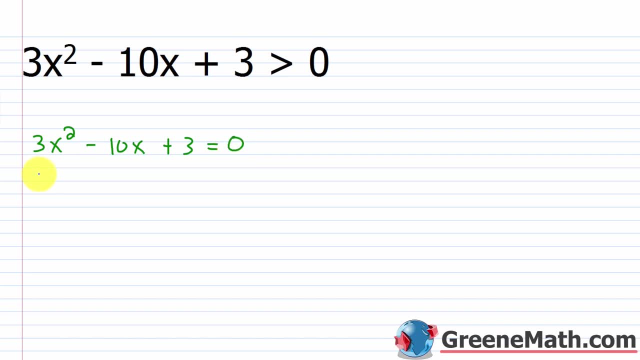 I can use my quadratic formula to solve this pretty easily. I just want the values for a, b and c. So a is 3, b is negative 10, and c is 3.. So we can say that x is equal to negative b. 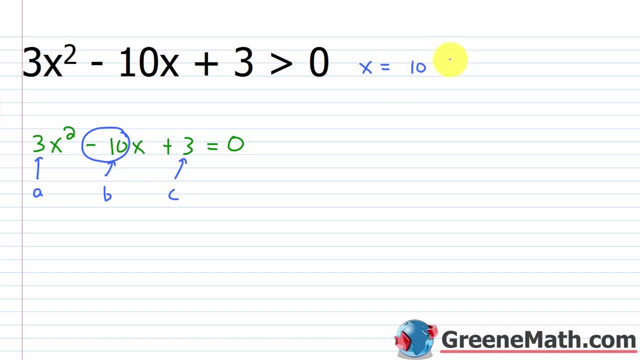 Here b is negative 10, so the negative of negative 10 is 10, plus or minus the square root of b squared Negative 10 squared is 100.. And then you have minus 4 times a times c. a is 3, c is 0.. 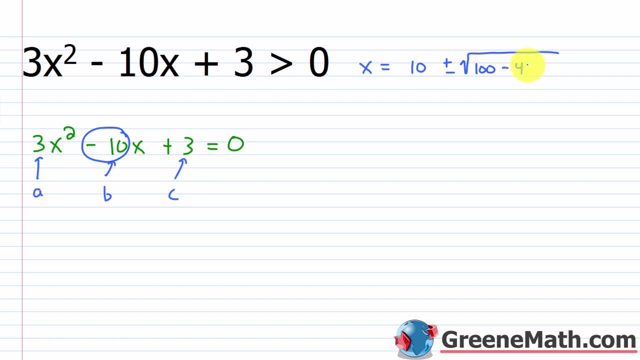 c is 3,, c is 3.. So you say 3 times 3 is 9,, so 4 times 9.. All right, so 4 times 9 is 36.. If I had 100 minus 36, that would be 64.. 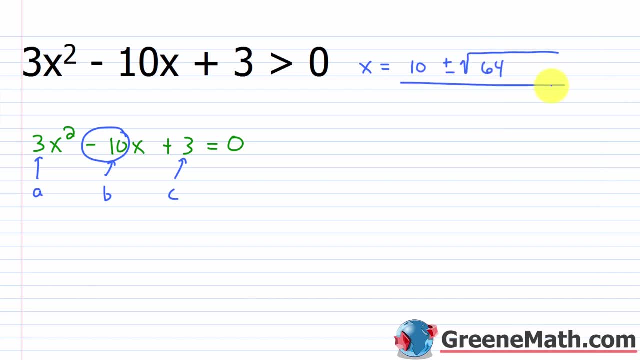 So this would be 64 here, and this is all over 2a. a here is 3,, so this is all over 6.. Square root of 64 is 8.. So this sets up two scenarios for us. We'll have: x is equal to 10 plus 8,. 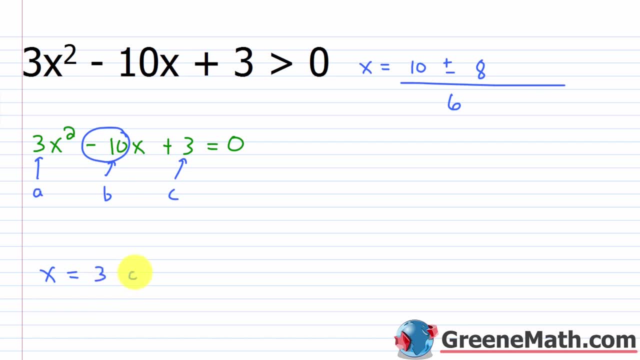 which is 18 over 6, so that's going to be x equals 3, or 10 minus 8,, which is 2 over 6.. 2 over 6 would reduce to 1 third, so x equals 1 third. 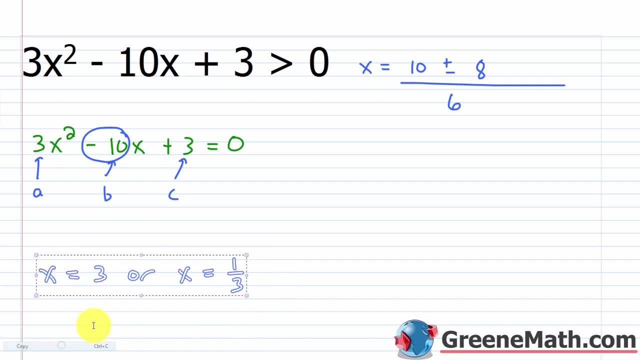 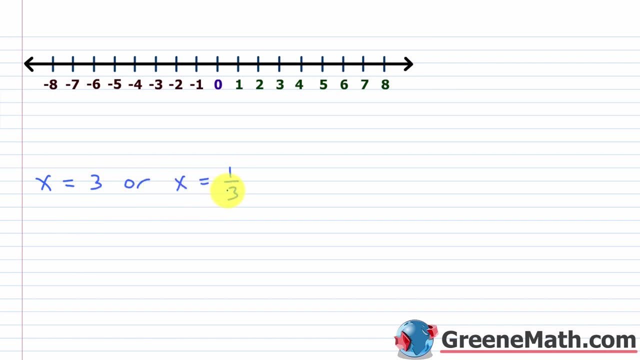 All right. so now we want to take these guys and bring them down to the number line, All right, so we're just going to paste the answers here. So we have x equals 3 or x equals 1, third. So the whole idea here is that. 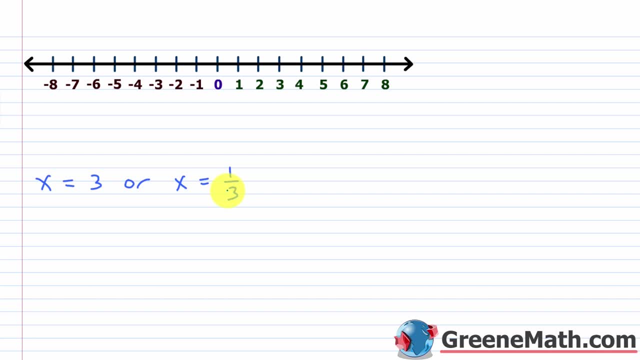 those answers are going to set up intervals for us. So at x equals 3, that's going to be an end point, So I can kind of circle 3, and you can draw just a little vertical line going down, And then at x equals 1 third, you do the same. 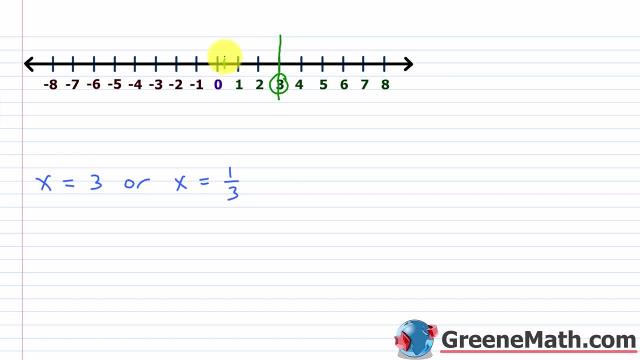 So I don't have a not for 1 third. I'd say it would be about right there. It doesn't need to be precise. You're just doing this for visual representation, So I can just kind of draw a vertical line there. 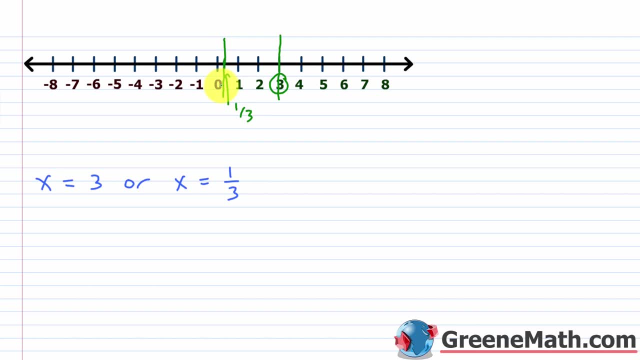 And essentially you now have three intervals here. So you have anything left of 1 third. So let's just call that interval a, just for talking. Then you have anything greater than 1 third but less than 3.. Let's call that interval b. 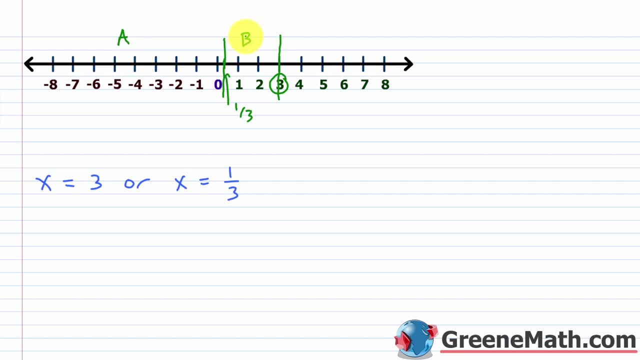 Then you have anything that's greater than 3.. Anything greater than 3.. So that's interval c. So now that I have these intervals set up, I can just grab test points from each interval see if they work. If they do work, that interval is in the solution set. 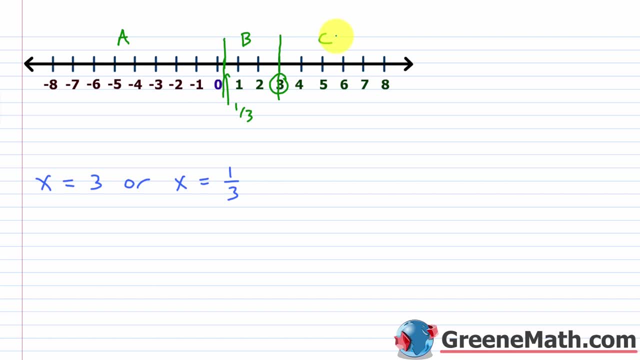 If they don't work, the interval is not in the solution set. So from interval a, the easiest number to grab would be 0.. So I'm going to go back up to my original inequality and I'm going to plug in a 0 for x. 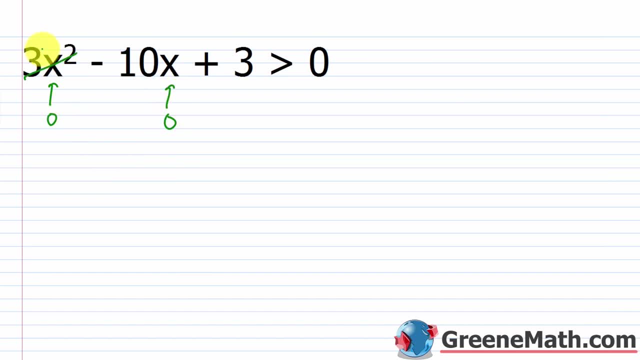 So a 0 there and there, What would happen? This is going to cancel. This is going to cancel. I'll have 3 is greater than 0. So we know that's going to work. So anything to the left of 1 third works as a solution. 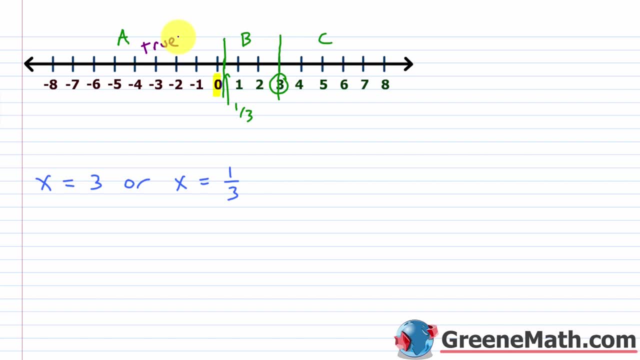 So I'll just write that this is true. This is true. Any value you plug in there would work. So what about this region where we have the capital letter b? So I can just choose something like 1.. A- 1 is in that interval. 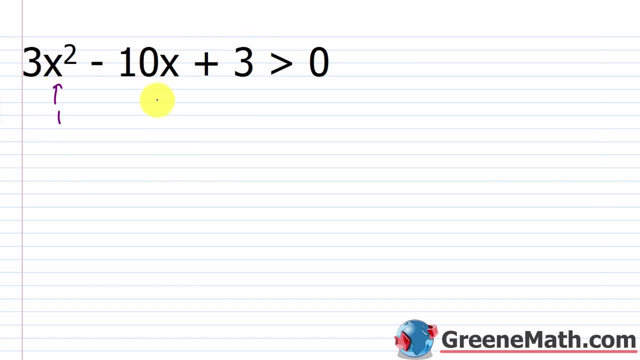 And if I plugged in a 1 for x, what would I get? So 1 squared is 1.. 3 times 1 is 3.. Minus 10 times 1 is 10.. Plus 3 is greater than 0.. 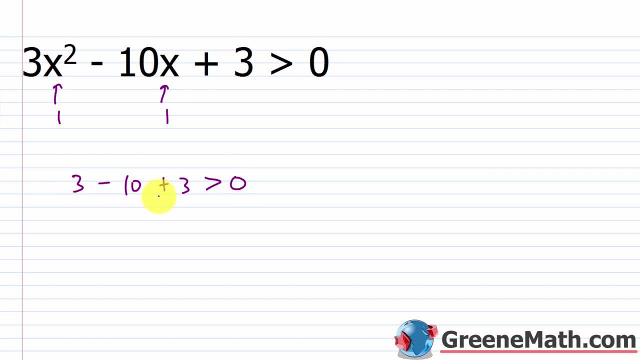 3 minus 10 is negative 7. Negative 7 plus 3 is negative 4. Is negative 4 greater than 0?? No, it is not, So that produces a false result, And so the values in this interval. we'll call it interval b again. 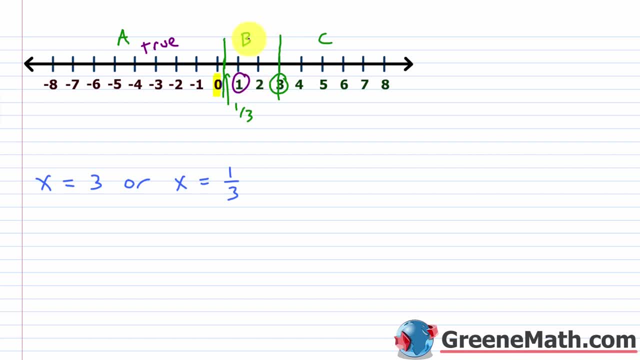 do not satisfy the inequality And so it's not going to be part of the solution set. So I'll write false here, False. Then what about interval c? Well, this is anything greater than 3. So I could just choose 4.. 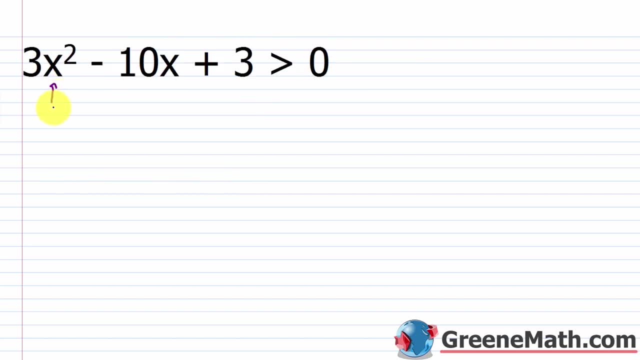 And we'll go back here and just plug in a 4 for every x. So 4 squared is 16.. 3 times 16 is 48.. Minus 10 times 4 is 40.. Plus 3 is greater than 0.. 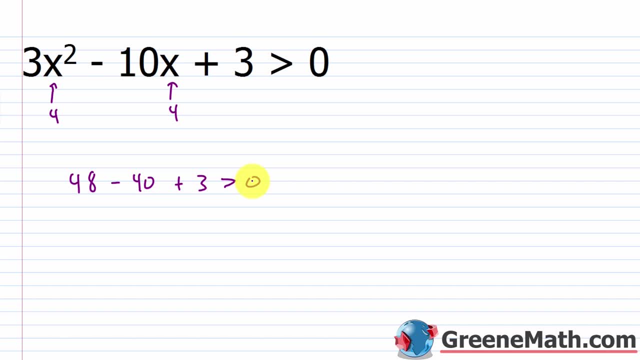 So 48 minus 40 is 8.. 8 plus 3 is 11.. 11 is greater than 0. So this results in a true statement. So we can go ahead and say that this is true over here, OK. 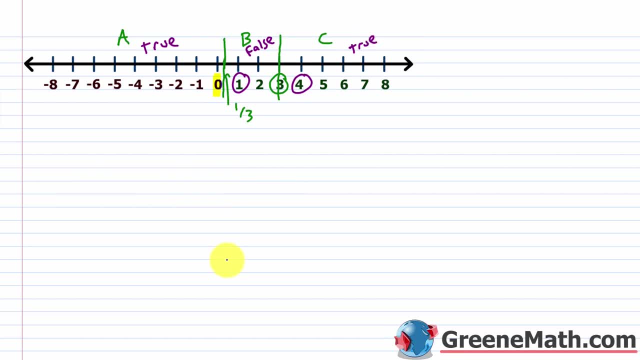 So let's erase this. We don't need this information anymore. So all I'm going to do is write my solution, And I can think about this graphically. I can think about it in interval notation. I can also think about it using set builder notation. 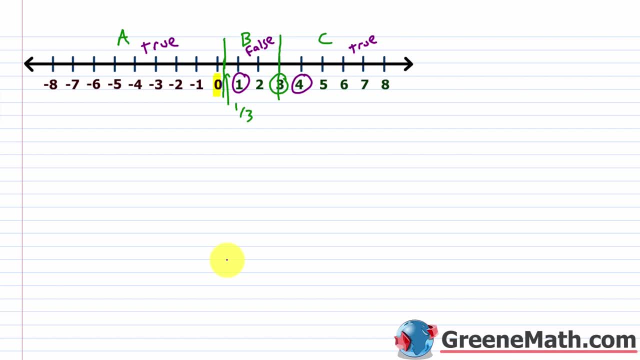 There's just lots and lots of ways to write the solution Graphically. I know that 1, third and 3 are not included. If I go back up, I have a strict inequality, So that means my endpoints will not be included. 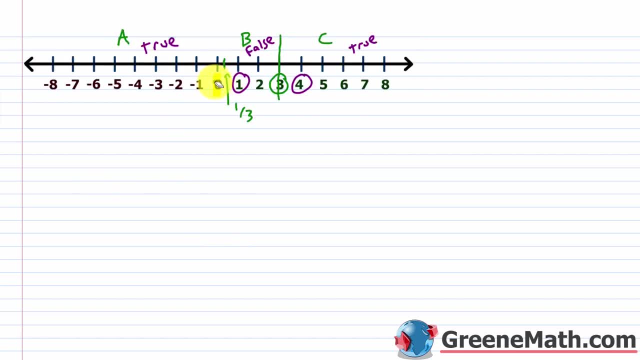 So I would put a parenthesis at 1 third facing to the left And I would shade everything to the left to indicate that, hey, 1 third doesn't work, but anything to the left of 1 third would work. Then at 3, I'm going to put a parenthesis facing to the right. 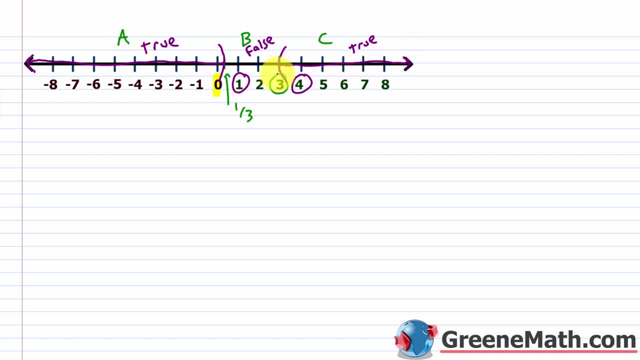 And then I'm going to shade everything to the right. So 3 doesn't work, but anything to the right of 3 would. Now that's the graphical solution. We saw that before back when we started solving a linear inequality in one variable. 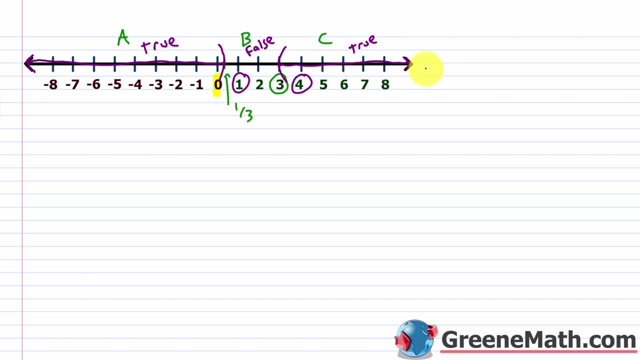 We've been doing this forever. And another thing we can do: we could use set builder notation So we could say the set of all x, such that we just list the conditions. So one condition is that x is less than 1 third. 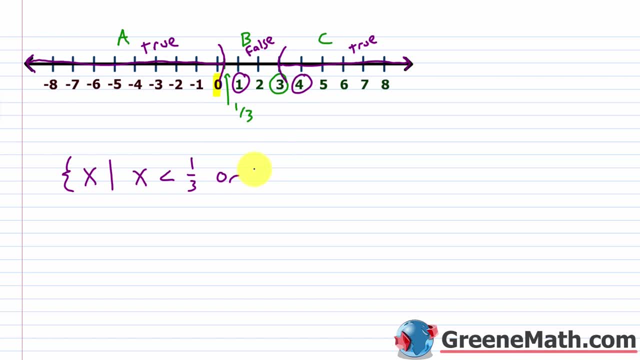 Then, or the other condition would be: x is greater than 3.. So any value we choose for x that's less than 1 third or greater than 3, will work as a solution in this inequality. Then another thing we can do, we could do interval notation. 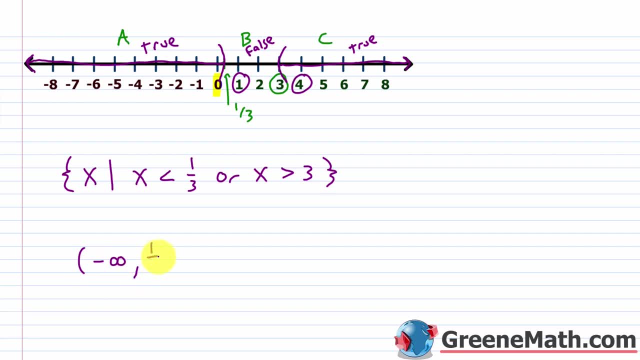 So from negative infinity up to infinity. So there's a set of x's that's less than 1 third or greater than 3.. Then the set of x's that's less than 1 third or greater than 3.. So that's going to be the union with the other set. 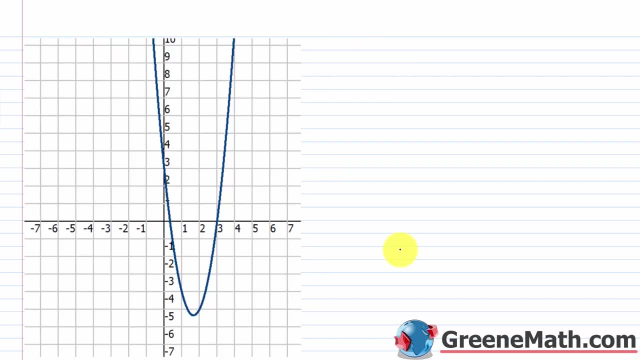 Which is not including 3, but anything larger. So before we kind of move on to the next problem, I want to demonstrate how you can go about solving this graphically. The first thing you would think about is you would think about just f of x or y is equal to 3x squared minus 10x plus 3.. 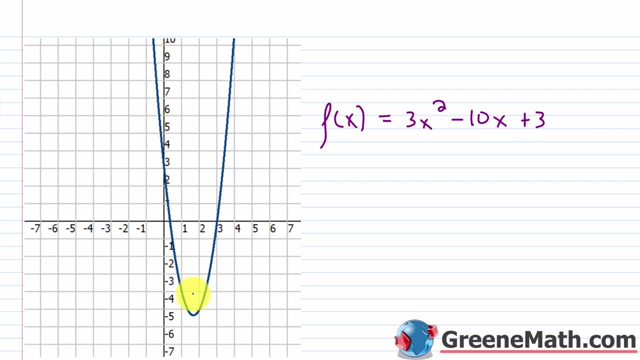 Say: OK, This produces this parabola right here. I would replace f of x with zero and I would solve: We know the solutions are: x equals three or x equals one-third. So that gives me an x-intercept that is three comma zero. 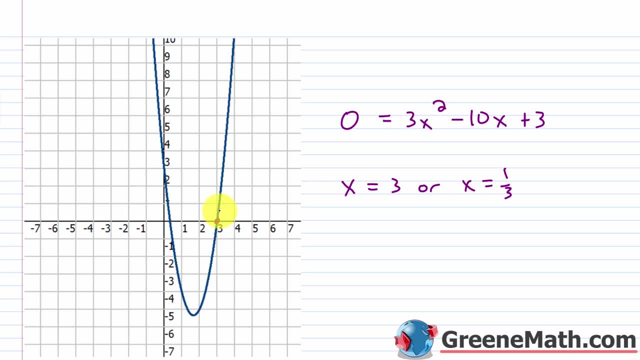 which is right here. And it gives me another x-intercept which is one-third comma zero, which is right here. So again, these x-intercepts will represent boundary points or places where you go from a solution region to a non-solution region. Right, It's separating the two. 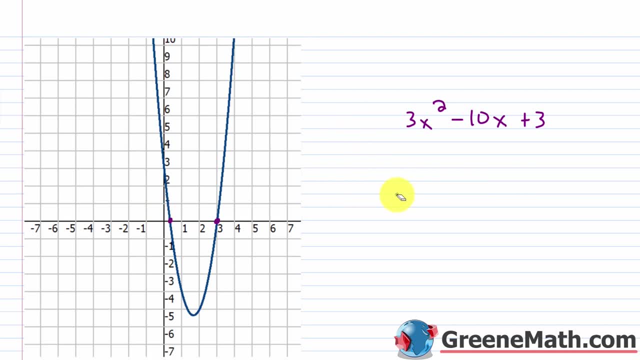 Now let me just scooch this down a little bit. Let me scooch this down. Let me just say: this is now greater than zero. So what am I asking for in this problem? graphically, I'm just asking for what x values make y or f of x greater than zero. Well, I can easily see that. 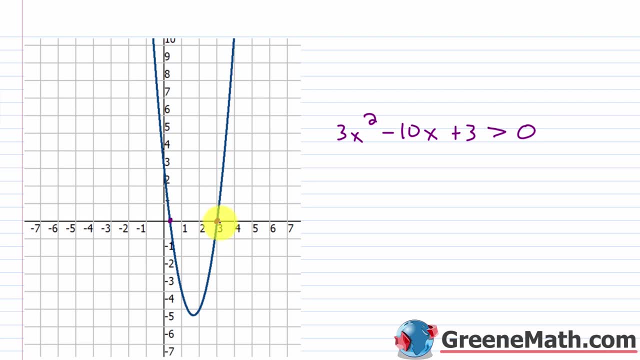 starting at three, but not three, right? Because an x value of three gives me a y-intercept. So I'm asking for what value of three gives me a y-intercept? value of zero? and zero is not included because it's a strict inequality. but anything to the. 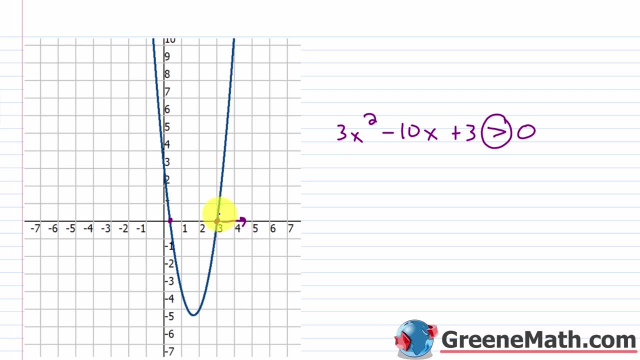 right of three. going this way, as we move, this way, we can see that the y values are larger than zero. it's the same thing over here. one third is not included because it makes y zero and again we have a strict inequality. but anything going to the left, right as x, gets smaller than one third. 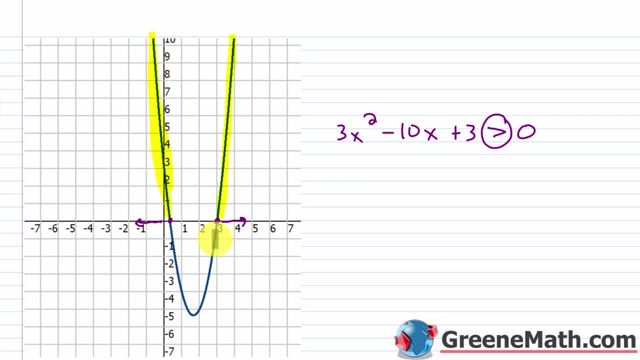 that's also going to give me a y value that's greater than zero. so this is a method you could theoretically use to solve this guy. i think it gives you a good insight to look at it a few times. but it's just not very practical, right if you had to take out graph paper and graph this guy and 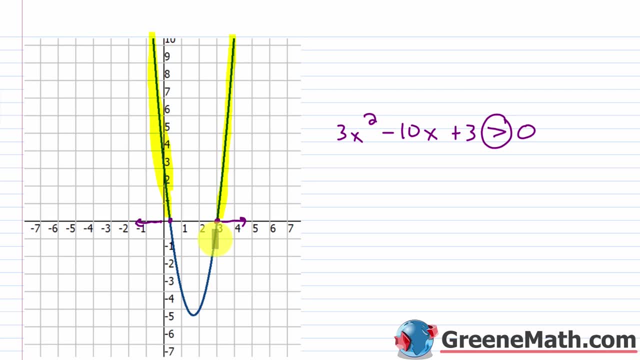 like set up a parabola. it's just a lot of extra work, right? maybe if you're using a graphing calculator, maybe if you're using software, it could be easier for you, but i think the method that we just used is much preferable to graphing. all right, let's take a look at one of the things that we're. 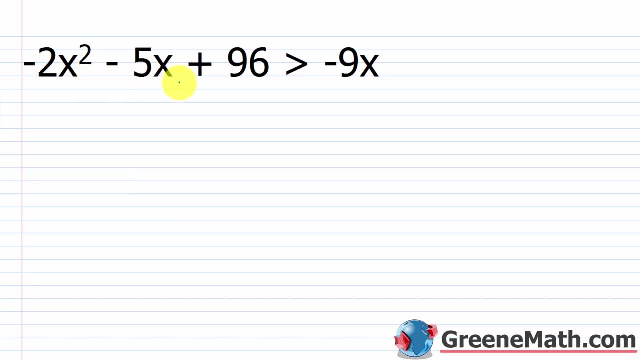 going to see now if we time size, it set that down and we add up the y racial one again. so what we've got is that if you're just guessing, we're not willing to use anything back to pass over. what we're going to end up with is this: two: cosine z, which is the norm de classical valuation. 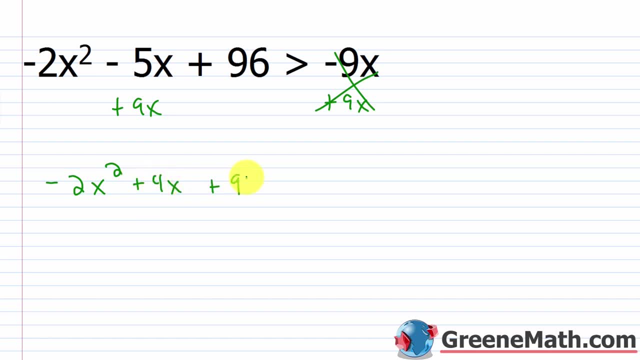 of a norm that the absolute value of y is minus two x squared. so let's say a 3000рав is sine, six times the norm in the form of u plus t. that says we're just going to take that form and do is this: and what's torn up we can cut the envelope and accepts. that's why we're going to have a. 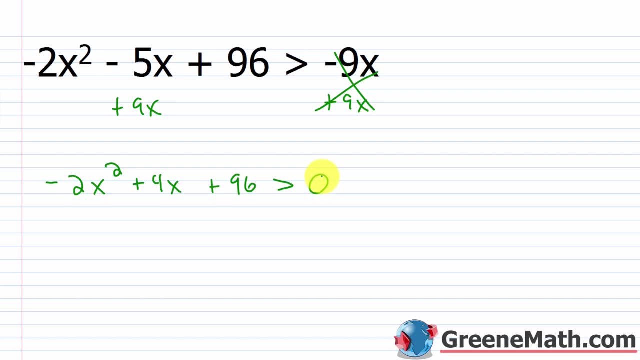 triangle here. so that's why we're making that back at it. all right, but instead of just doing и, we can divide both sides of the inequality by 2 or negative 2.. But if we're dividing by negative 2, remember we have to flip the direction of the inequality symbol. 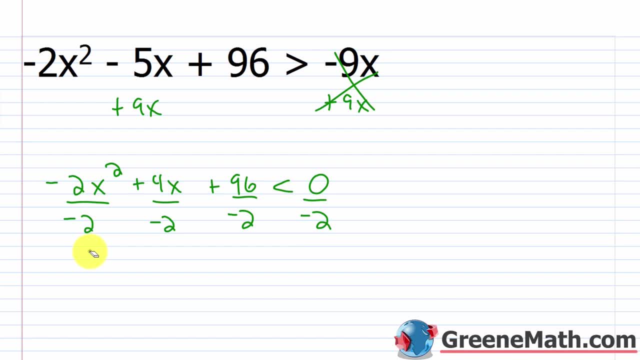 So this would now be a less than. So. this would be x squared minus 2x, So minus 2x, And then 96 over negative 2 is 48. So minus 48. And this is now less than 0 over negative 2,. 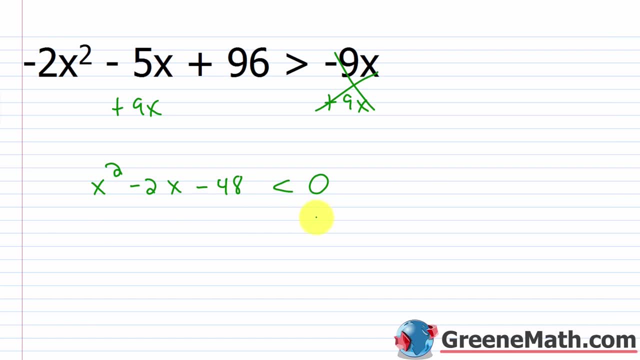 which is 0.. All right, So this is going to be the inequality we're working with here, And I'm just going to change this into an equation. So I'll change this into: x squared minus 2x minus 48 is equal to 0.. 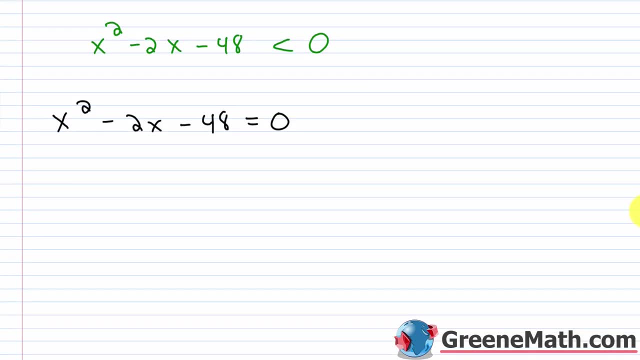 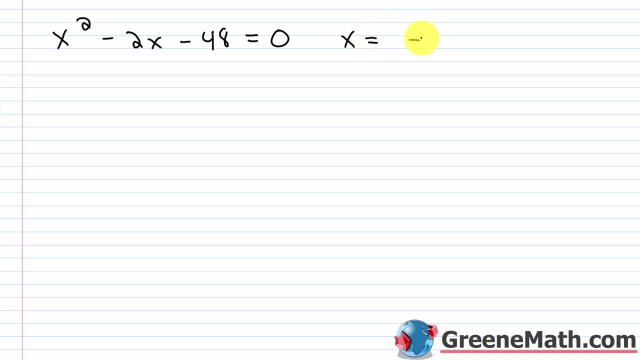 I can easily solve this using factoring, Or you can use the quadratic formula. It doesn't really matter, Let's just go ahead and use the quadratic formula so that we're consistent. So x equals negative b. In this case, b is negative 2.. 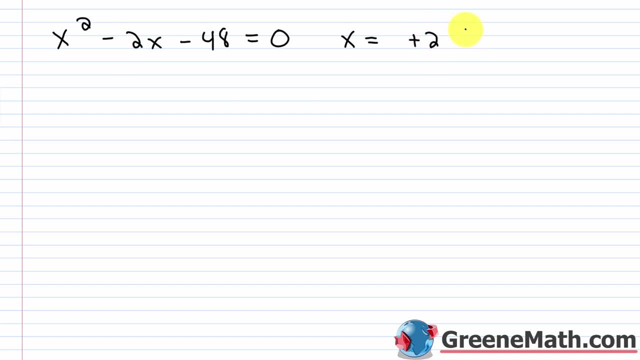 So the negative of negative 2 is positive 2.. Plus or minus the square root of b squared, Negative 2 squared is 4.. Minus 4 times a, a is 1 here. So times 1 times c, c is negative 48.. 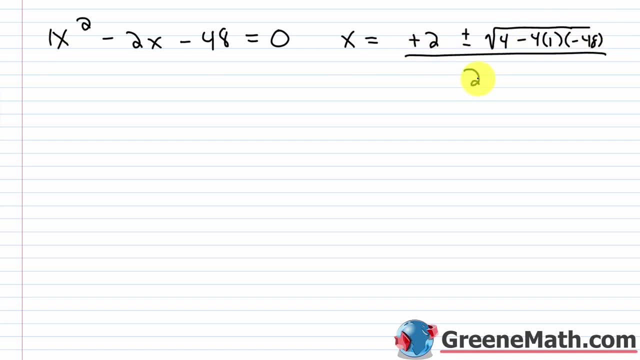 Okay, This is all over. 2a. a is 1.. So just over 2.. So the easiest way to do this is: just think about this as plus negative 4 here. So negative 4 times negative 48 is 192.. 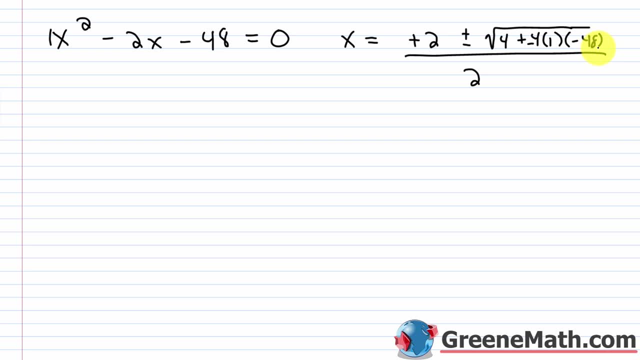 So you would have 4 plus 192, which is 196.. And the square root of 196 is 14.. So this would be 14 here. So my two solutions would be: x is equal to 2 plus 14 is 16.. 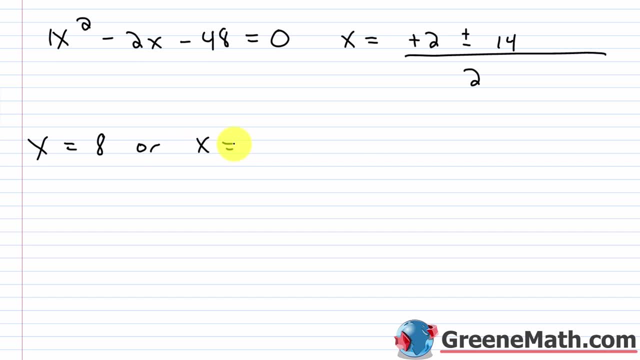 16 divided by 2 is 8. Or x is equal to 2 minus 14 is negative 12.. Negative 12 divided by 2 is negative 6.. So x either equals 8 or x equals negative 6.. Okay. 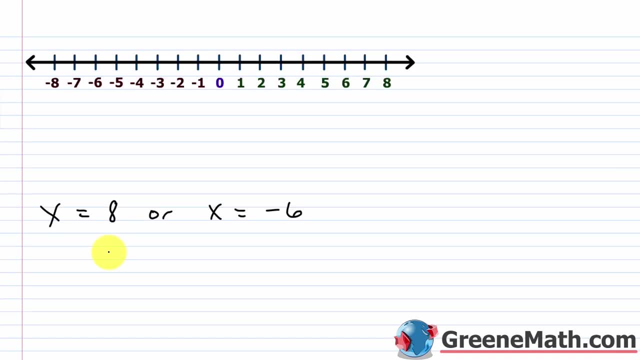 So let's take this down to the number line. Okay, So we have x equals 8. So 8 is right here, And then x equals negative 6. So that's right here. So again, just draw yourself a little vertical line at each end point. 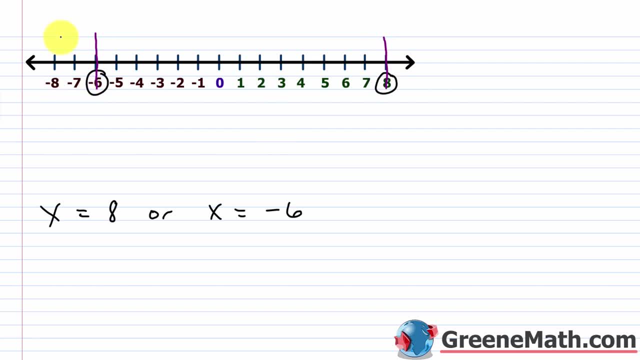 And you're dividing the number line into region. So left of negative 6, we'll call that region a, or interval a Between negative 6 and 8, we'll call that interval b, And then to the right of 8,. 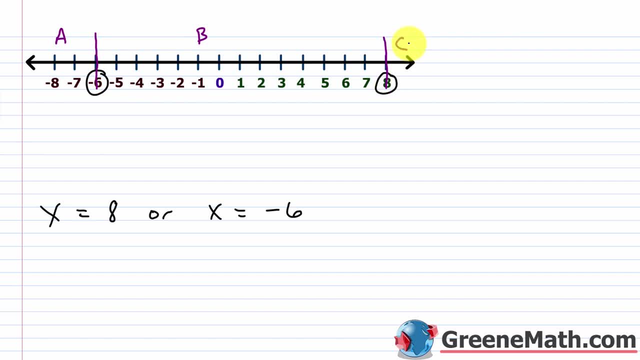 we'll call that interval c. So in interval a let's just pick negative 7.. So does negative 7 work as a solution? So plug in a negative 7 here And here and here. Negative 7 squared is 49.. 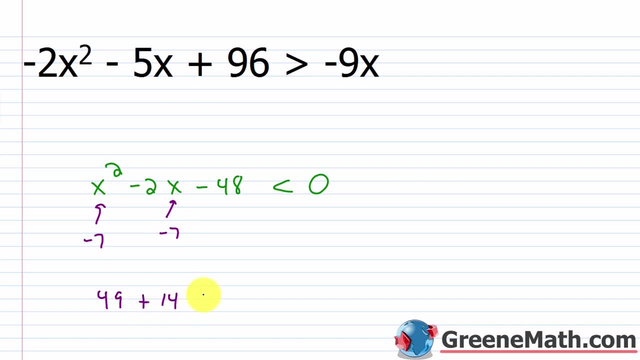 Then you'd have negative 2 times negative, 7, which is plus 14, and then minus 48. So is this less than 0?? We know without even doing the problem, it's not. 49 minus 48 would be 1.. 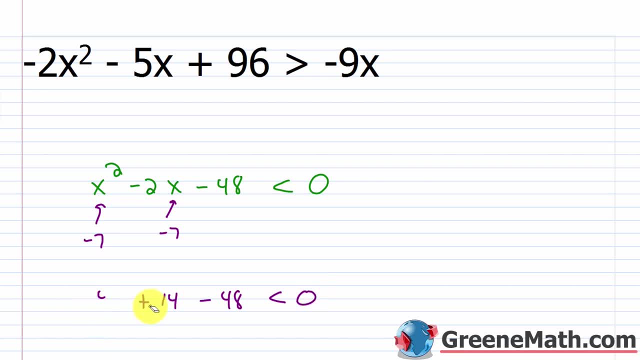 1 plus 14 is 15.. So we know that 15 is not less than 0.. So that's false. So we can say this is false. Then what can we say about this interval or region b? We can just choose 0.. 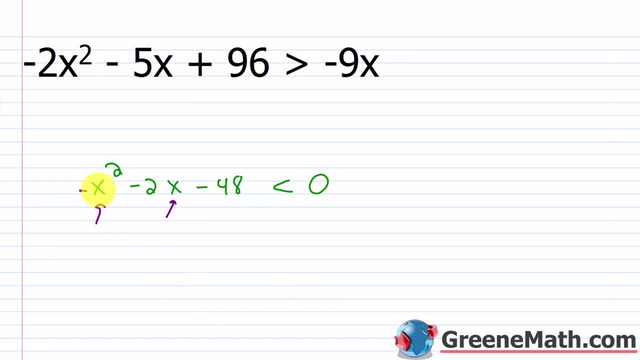 And if we plugged in a 0 for x- we know that this would go away- You'd have negative. 48 is less than 0. That's true. So this is true. And then for region c, we could just choose 9.. 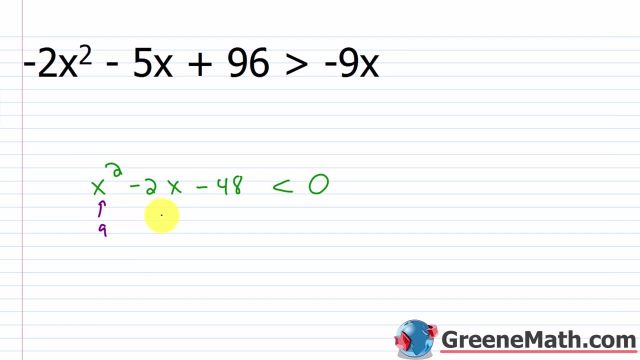 So if I plugged in a 9 for x, I plugged in a 9 for x- 9 squared is 81. Then negative 2 times 9 would be minus 18, and then minus 48, and this is less than 0.. 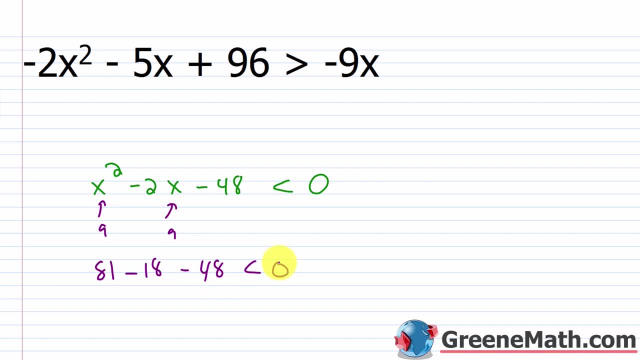 81 minus 81 is 1.. Minus 18 is 63.. 63 minus 48 is 15.. So 15, again is not less than 0. So anything in region c would fail. So this is false. 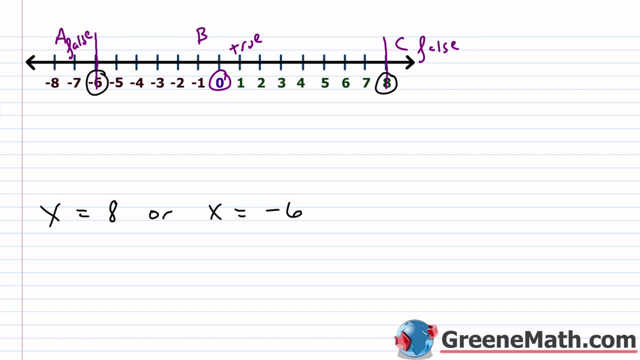 Now you're working with a strict inequality here, So your endpoints or your boundary points are not gonna be included. So graphically, I would put a parenthesis at negative 6 facing to the right and a parenthesis at 8 facing to the left. 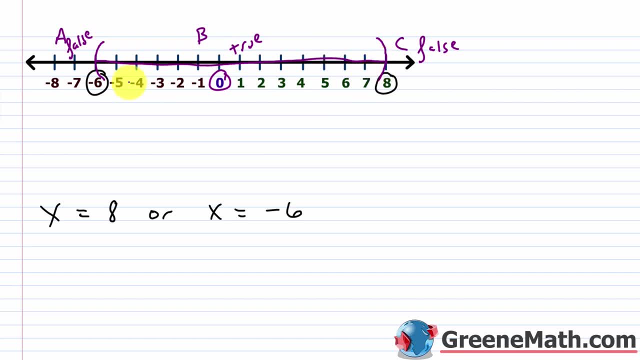 and I would just shade everything in between. So anything larger than negative 6, up to but not including 8, would work as a solution for that inequality. So in set builder notation we could say the set of all x, such that x. 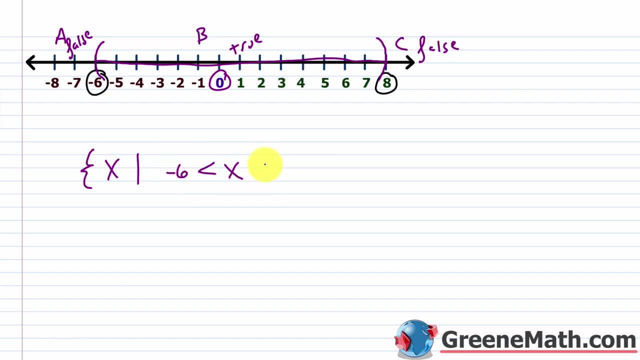 is greater than negative 6 and less than 8.. And then, to kind of wrap this up, I'm just gonna use interval notation. I'm gonna have a parenthesis- negative 6, and then up to, but not including, 8,, so another parenthesis. 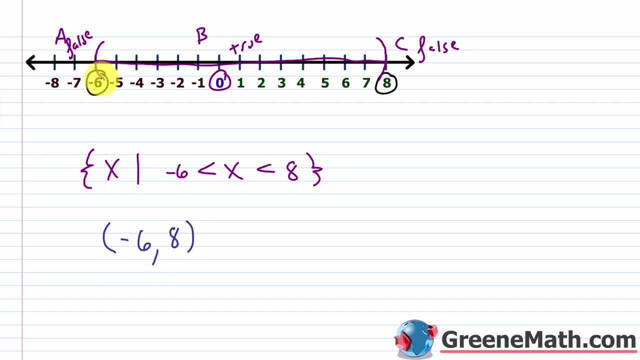 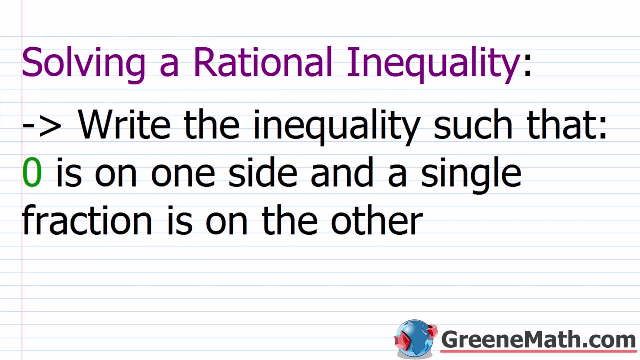 So this is my interval. Again: anything larger than negative 6, up to, but not including 8.. All right, so now let's talk a little bit about how to solve a rational inequality. So with a rational inequality you're really just thinking about the exception here. 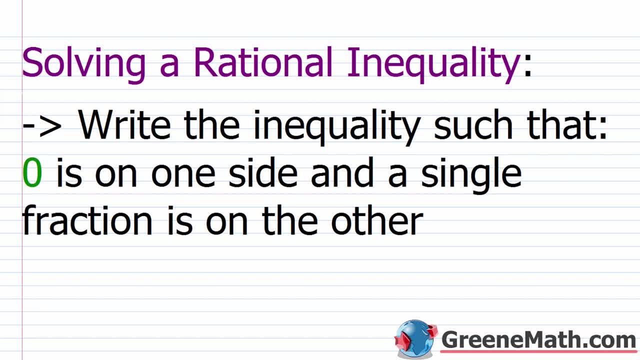 where the denominator is made into 0. Remember, we can never divide by 0. So that's the one thing that you really gotta pay attention to here. Everything else is pretty similar. So the first thing is to write the inequality such that: 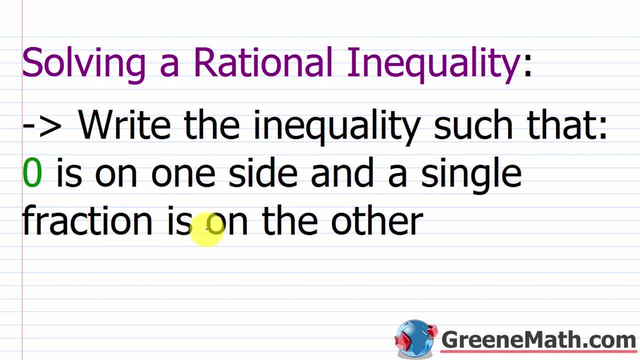 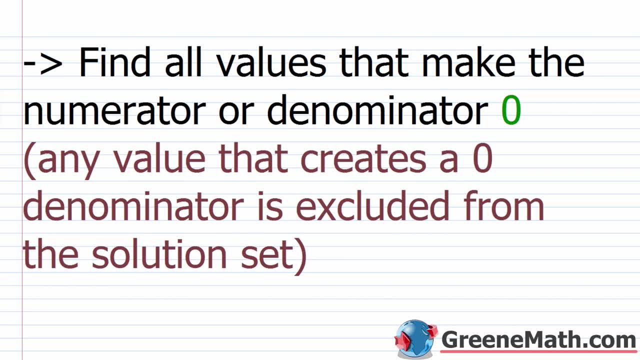 0 is on one side and a single fraction is on the other, Then once you've done that, you're gonna find all values that make the numerator or denominator, 0. So I'll take the numerator, I'll set it equal to 0, and I'll solve it. 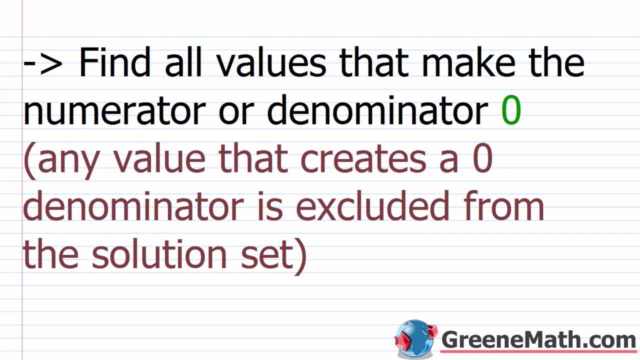 I'll take the denominator, I'll set it equal to 0, and I'll solve it. Now. any value that creates a 0 denominator is excluded from the solution set, Excluded from the solution set In the case where you have a value. 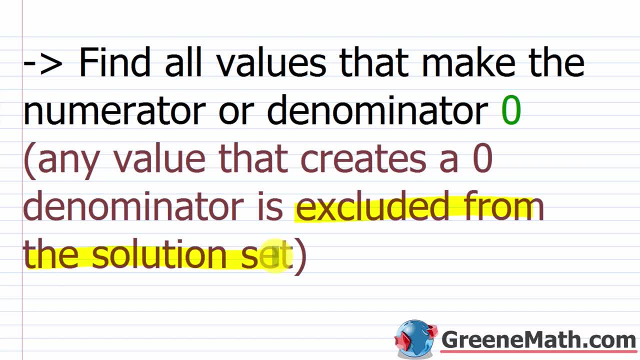 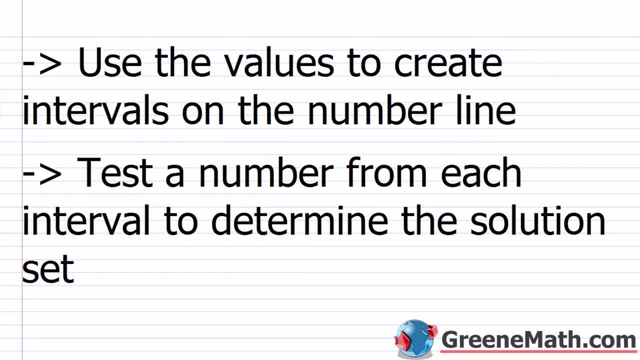 that makes the numerator equal to 0, you have again. you've got an endpoint there, so you've gotta pay attention to whether it's a strict inequality or a non-strict inequality. All right, so again we're using the solutions that we got. 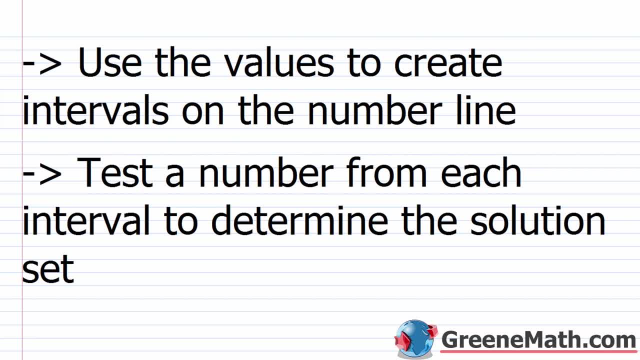 or the values to create intervals on the number line. Again, these are gonna be our endpoints or our boundary points, And we're just gonna test the number from each interval to determine the solution set. So very similar to what we just did. Again, we just have to remember that we can't divide by 0.. So, as a last point, we have here that endpoint: we can't divide by 0.. So, as a last point, we have here that endpoint: we can't divide by 0.. So, as a last point, we have here that endpoint. 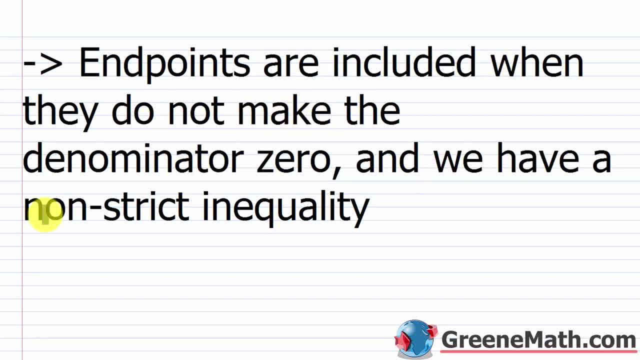 we can't divide by 0. And we have a non-strict inequality. So if you have a strict inequality, they're never included. If you have a non-strict inequality, they're included only in the circumstance that they do not make the denominator 0. 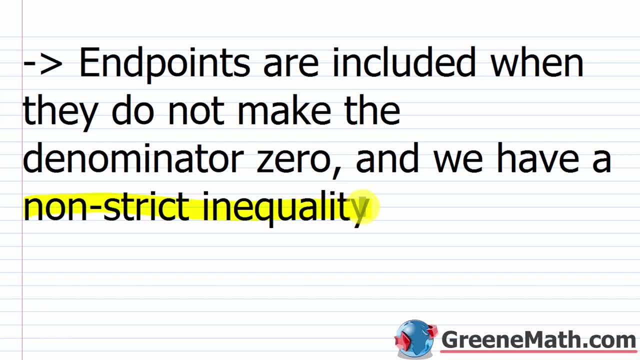 If you put something in there that makes the denominator 0, you're gonna get the wrong answer. okay, It's a common mistake because you go from quadratic inequalities to rational inequalities in the same section. You get used to: oh, I have a non-strict inequality. 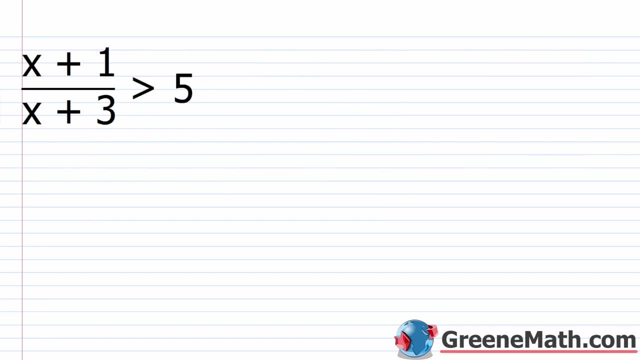 so I throw it in my answer and then it's wrong. All right, let's look at the first example. So we have x plus 1 over x plus 3, and this is greater than 5.. So the very first thing I'm gonna do, 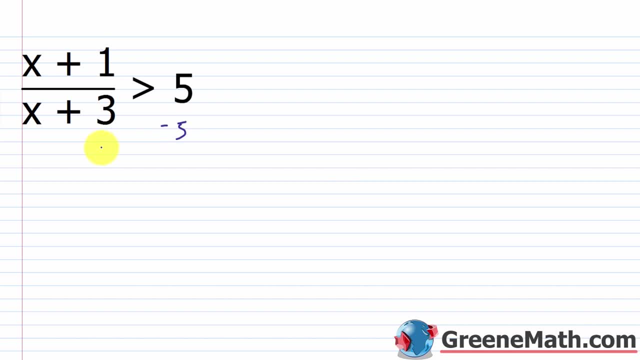 I'm gonna subtract 5 away from each side of the inequality, So I will have x plus 1 over x plus 3, and this is minus 5, and this is greater than 0. now, So how do I write this as a single fraction? 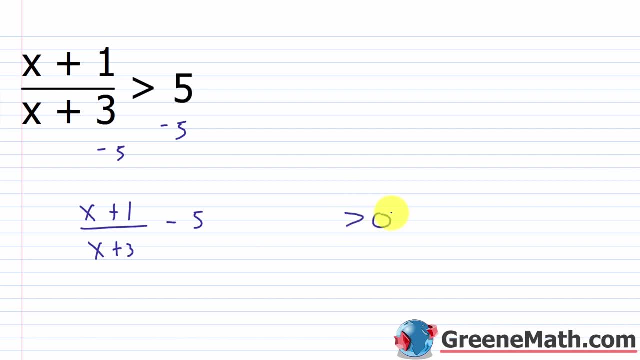 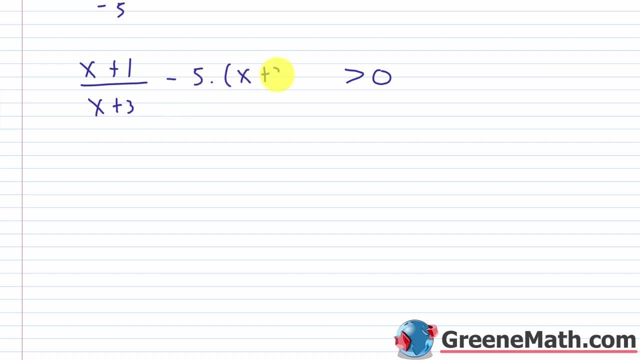 Well, I just need to get a common denominator going. So let me kind of move this down a little bit, Let me kind of scooch down, get some room going To get a common denominator. I would just multiply this by the quantity x plus 3. 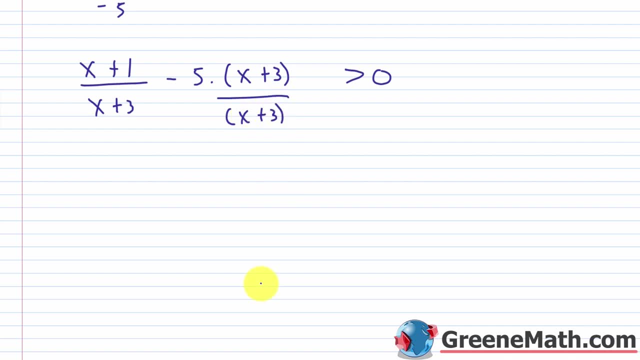 over the quantity x plus 3.. Very easy, So I would have x plus 1, and then negative 5 times x would be minus 5x, and then negative 5 times 3 would be minus 15.. This is over the common denominator of x plus 3.. 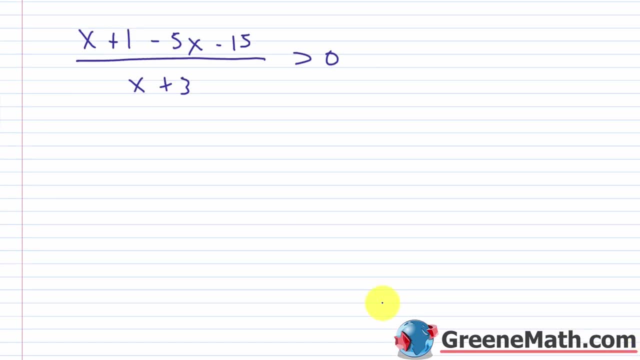 Of course this is greater than 0. So in the numerator if we combine like terms: x minus 5x is negative 4x, and then 1 minus 15 is negative 14.. So you would have negative 4x minus 14,. 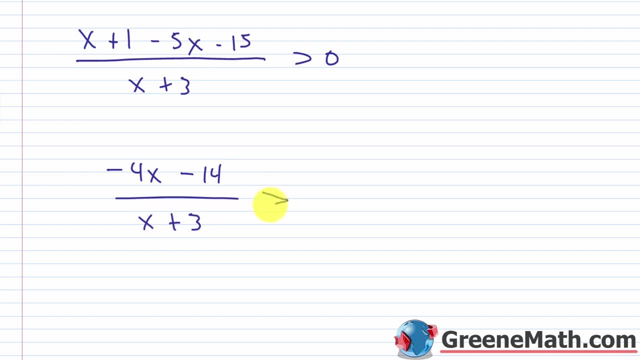 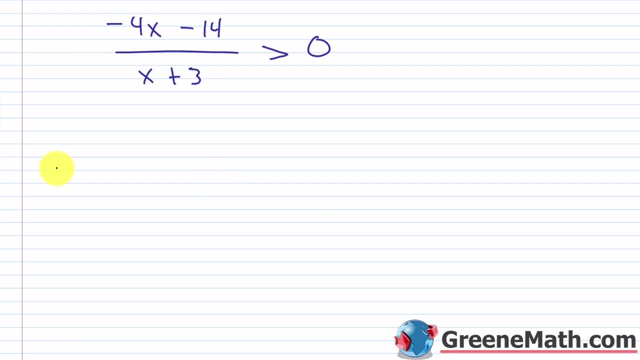 and this is over x plus 3, and again this is greater than 0.. Now what I want to do? I wanna take the numerator and I wanna set it equal to 0.. So negative 4x minus 14 is equal to 0. 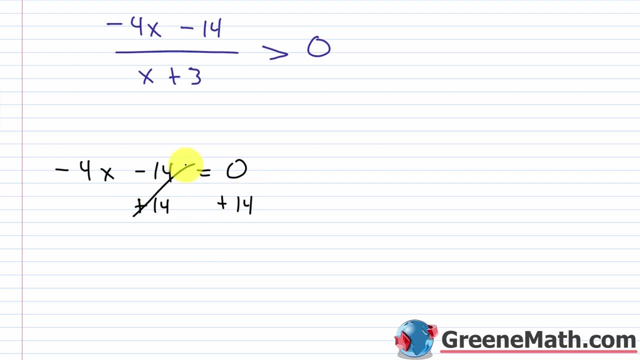 Okay, so I would just add 14 to each side of the equation here. That's gone. I'll have negative. 4x is equal to 14.. Divide both sides by negative 4.. That'll cancel. with that, I'll have x is equal to. 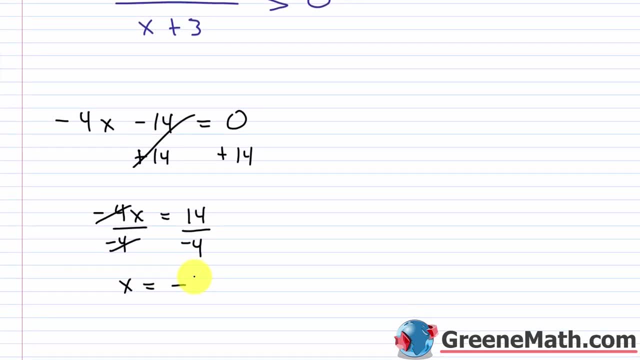 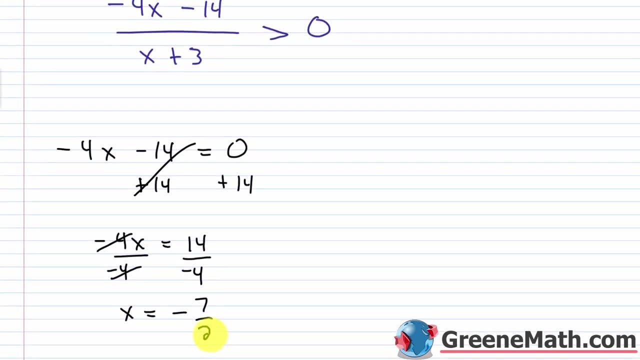 we know this would be negative. 14 is divisible by 2, and so is 4.. So 14 divided by 2 is 7.. 4 divided by 2 is 2.. So this would be negative. 7 halves. 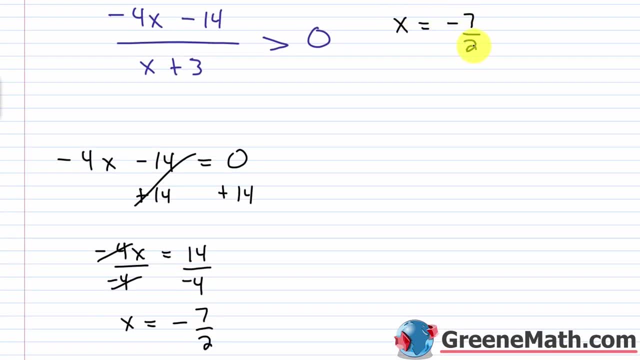 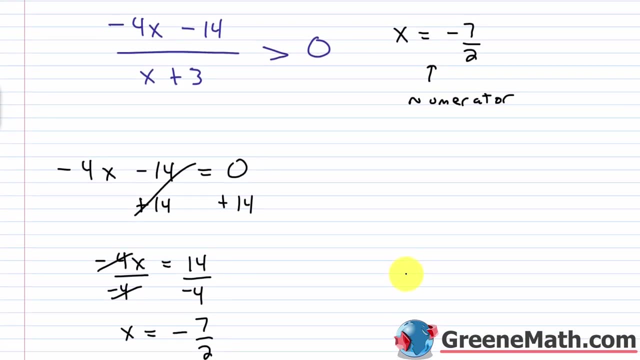 So x equals negative 7 halves. That's gonna be one end point and that's gonna be from the numerator. So the other end point's gonna come from setting x plus 3 equal to 0.. In this case I could just subtract 3 away. 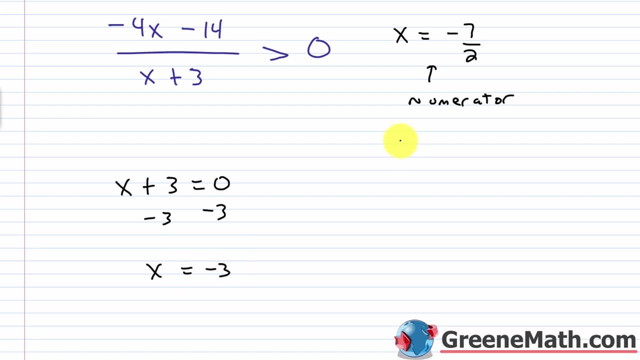 from each side of the equation I get x equals negative 3. So x equals negative 3. This comes from the denominator. Now, in this case I have a strict inequality, So neither end point will be a solution. But in the case where it's a non-strict inequality, 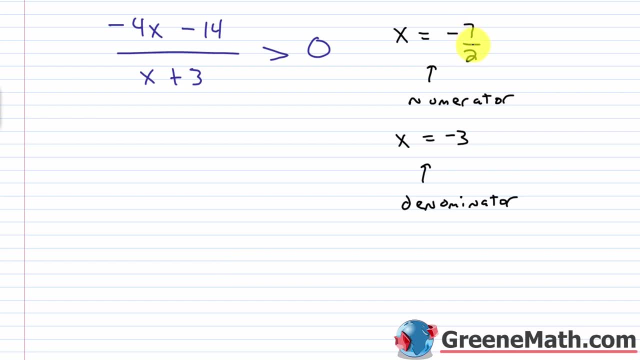 I can take negative 3 and take 2.. negative seven halves and it would be a solution, right? Because you think about the fact that if this was a greater than or equal to, if I plugged in a negative seven halves for x, the top part. 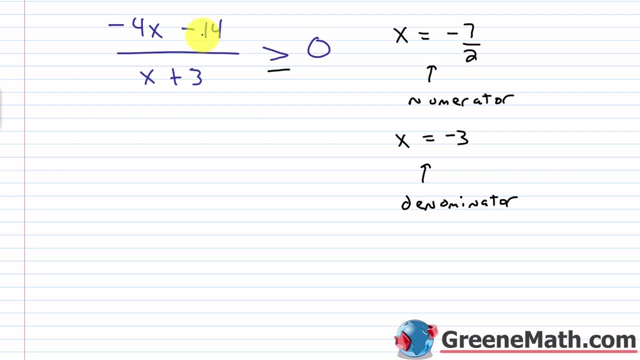 would become zero. Zero divided by anything other than zero would give me zero, So I would get: zero is greater than or equal to zero, which would be true. right, Zero equals zero. But because I pull this away and make this a strict inequality, this will not satisfy the inequality, So it's not part. 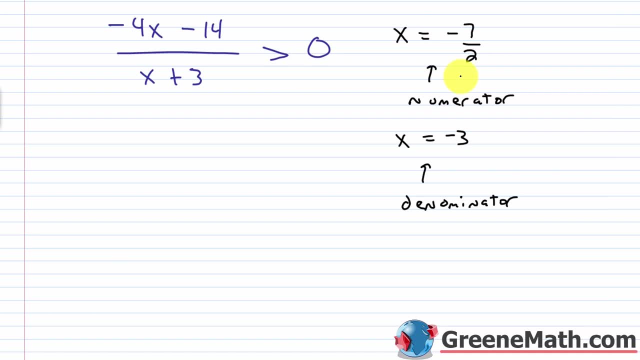 of the solution set. The x equals negative three will never be part of the solution set because if I plug in a negative three down here, I get negative three plus three, which is zero, and I cannot divide by zero. So it's very important that you pay attention to what's. 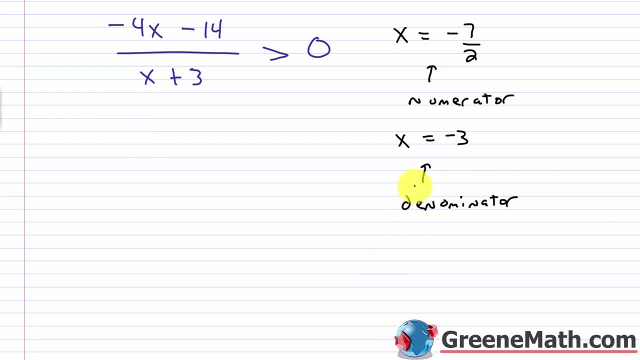 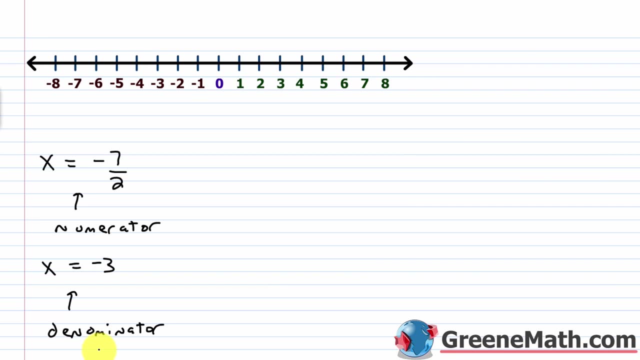 going on. I always tell my students to label where everything came from so you don't forget. So let's copy this. And so these are going to be my end points. So negative three is right here- Let's make a little vertical line there- And negative seven halves- where's that going to be? 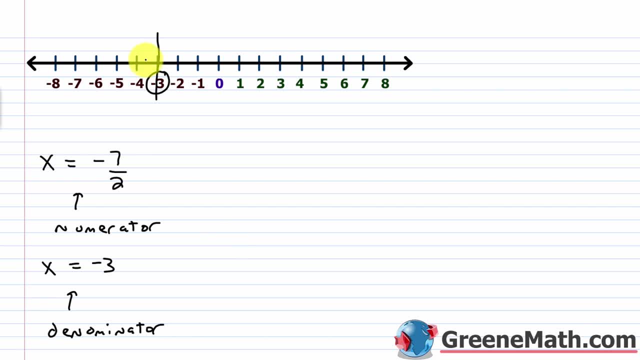 Well, it's negative 3.5, really, if we thought about it. So it's about halfway between negative three and negative four. So let's say it's about right there. Let's say this is negative seven halves. Let's make another vertical line there. So it's going to set up a kind of small region. 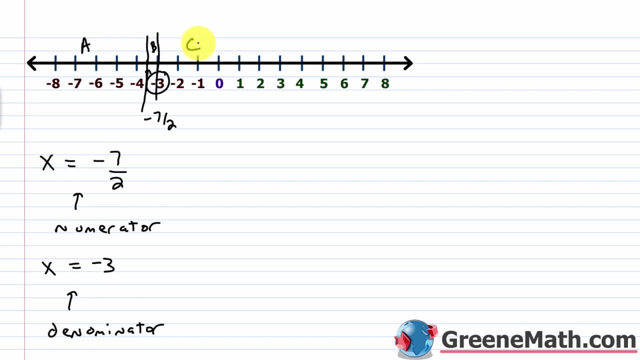 Let's say this is region A, this is B and this is C. So in region A, let's pick something easy. Let's just take negative five. So I'm going to plug back in for x in the original inequality. so I'm going to plug in a negative five there and there. So negative five plus one is negative four. 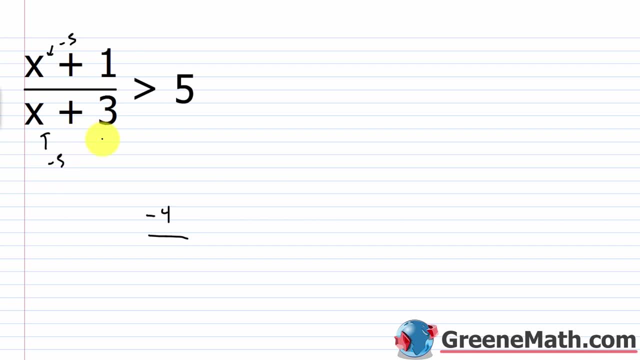 So you'd have negative four over negative five plus three is negative two, So this is supposed to be greater than five. Negative four divided by negative two is positive two, So is two greater than five? No, So this would be false. This is false. We can say this one was false, Okay. 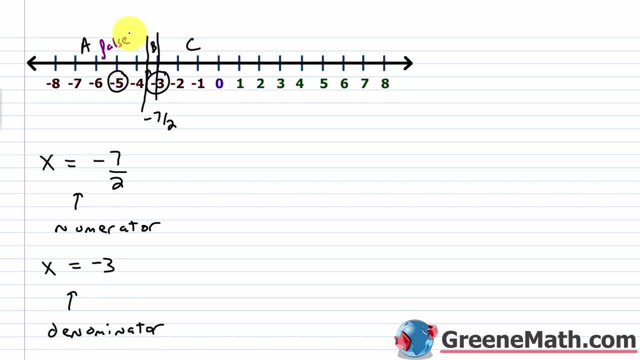 so it's a pretty narrow region Where we have between negative three and basically negative 3.5.. But we can use negative 3.25 because that would lie between those two. So let's go back up and let's say we have negative. 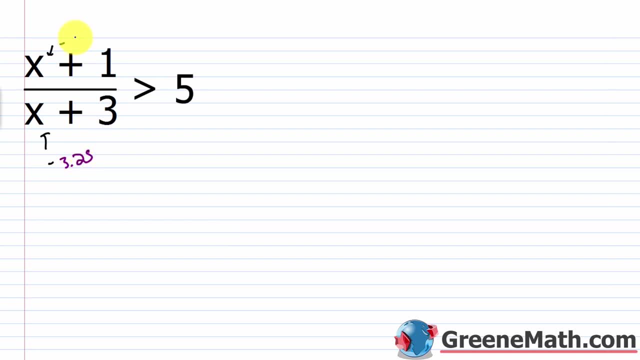 3.25.. So negative 3.25.. So negative 3.25 plus one would be negative 2.25.. Then this is over Negative 3.25 plus three. So this would be negative 2.25.. If I divided negative 2.25 by negative 0.25, I would get. 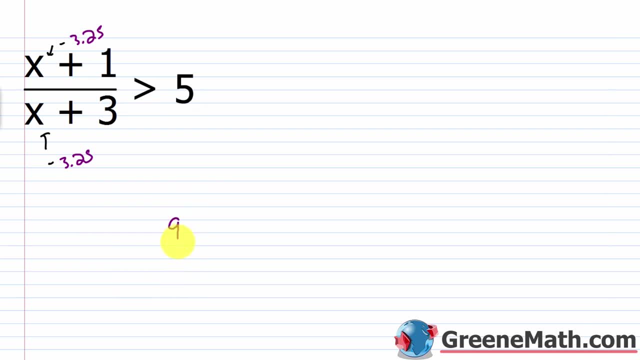 nine. So this would be nine is greater than five, which is true. So for region B, I could say: this is true. Then for region C, let's just pick zero. If I plugged in a zero for x, what would I get? So zero there and a zero there. Essentially, these are gone. You'd have 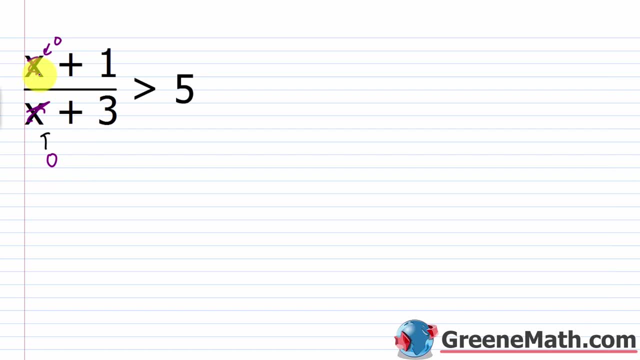 1. 3rd, You have 1 over 3, which is not greater than 5, so that's false. So this is going to be false, And so we're ready to give our solution. We know that the endpoints negative 7 halves and. 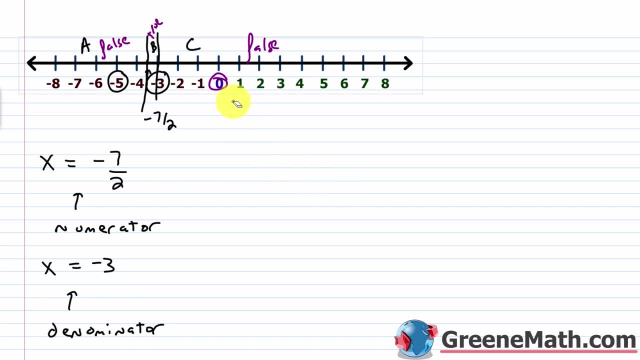 negative 3 are not included. So essentially, all we would have here is we would graph a parenthesis here at negative 3.5 or negative 7 halves facing to the right, and a parenthesis here at negative 3 facing to the left, and then we would just graph everything in between. 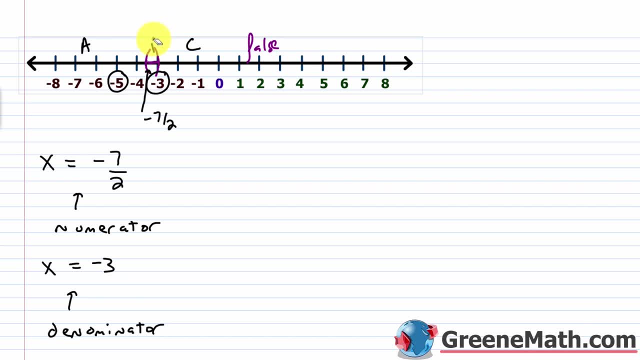 So that's your graphical solution. I can erase the false and true and the a and the b and the c. I don't need any of that anymore. And we can say that in solution set notation we can say the set of all x, such that x is greater than negative 7 halves and x is less than negative 3.. And then 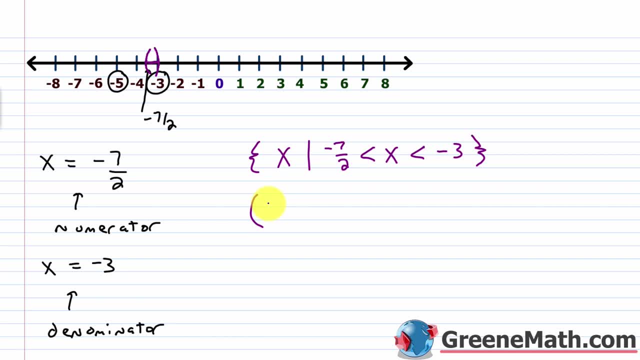 lastly, if we were to use interval notation, put a parenthesis, Negative 7 halves comma, you would have negative 3 and then a parenthesis. All right, pretty easy overall. Let's just look at one more to kind of wrap things up. We have x minus 2 over x plus 2,. 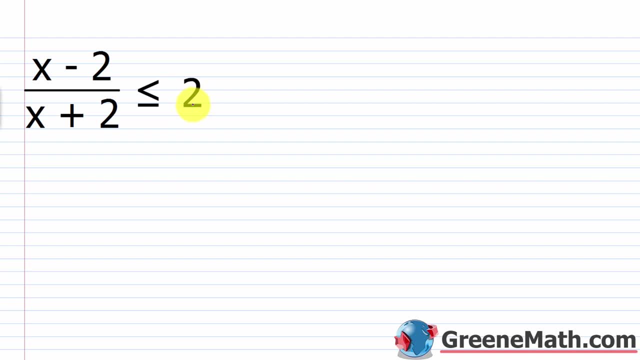 and this is less than or equal to 2.. So again, I want one single fraction on one side and then I want 0 on the other. So I'm going to add negative 2 to both sides or subtract 2 away. 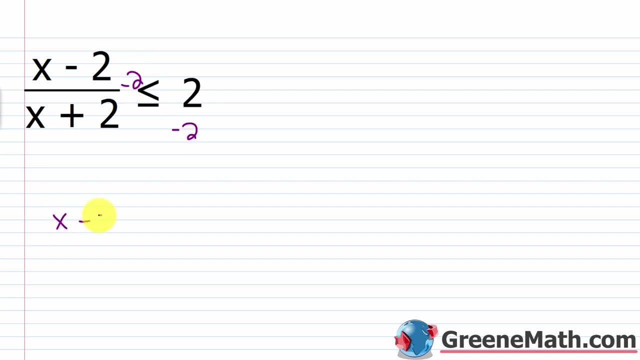 however you want to think about that. So I'll have x minus 2 over x plus 2,, then minus 2, or I could put plus negative 2, or again, however you want to think about that, This is less than or equal to 0. So they get a common. 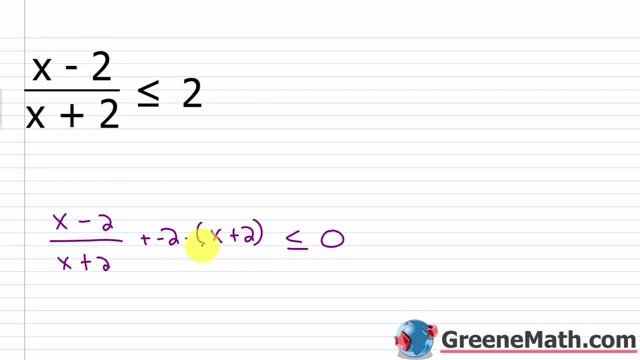 denominator. I'll multiply this by the quantity x plus 2 over x plus 2.. And what that's going to give me I'll have x minus 2, and then negative 2 times x. so minus 2x and then negative 2 times. 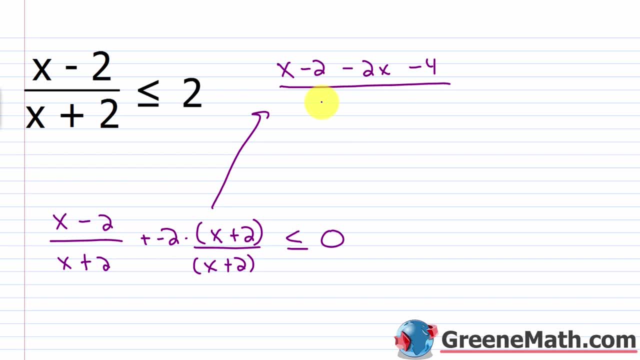 2, so minus 4, over the common denominator of x plus 2, and this is less than or equal to 0.. So x minus 2x is negative x, and then negative 2 minus 4 is negative 6.. So you have negative x. 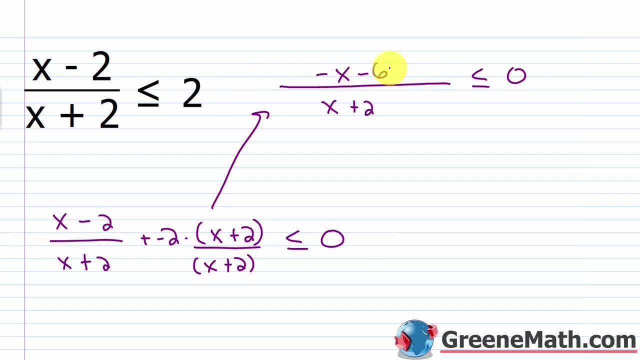 minus 6.. Negative x minus 6, this is over x plus 2, and this is less than or equal to 0.. Okay, so pretty easy to get to that point. And then again, all I want to do? take my numerator, which in this case is negative x minus 6, set it equal to 0. I could solve this. 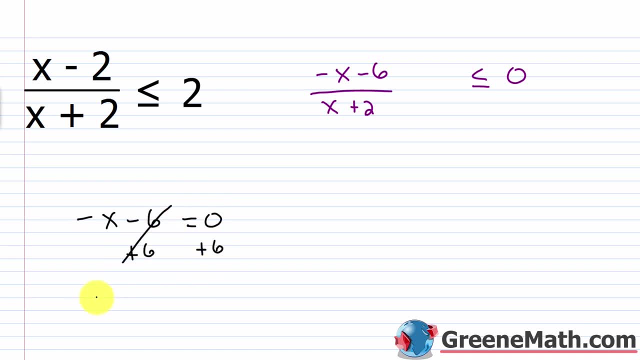 by adding 6 to each side of the equation. That would go away. I'd have negative. x is equal to 6, multiply both sides by negative 1, you get x is equal to negative 6.. So for the numerator. for the numerator, x is equal to negative 6.. Okay for the denominator. 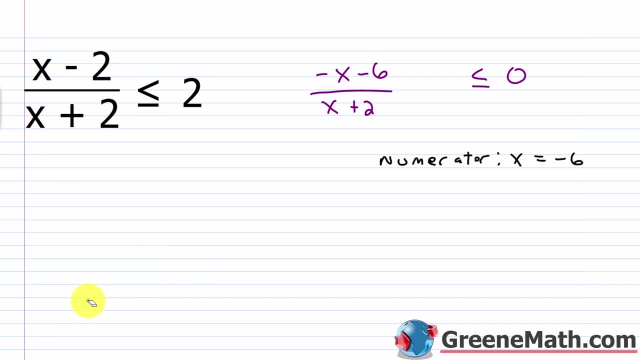 we have x plus 2.. So x plus 2 is equal to 0.. Subtract 2 away from each side of the equation, you get x equals negative 2.. So for the denominator x equals negative 2.. So in this case we have a non-strict inequality. You have less than or. 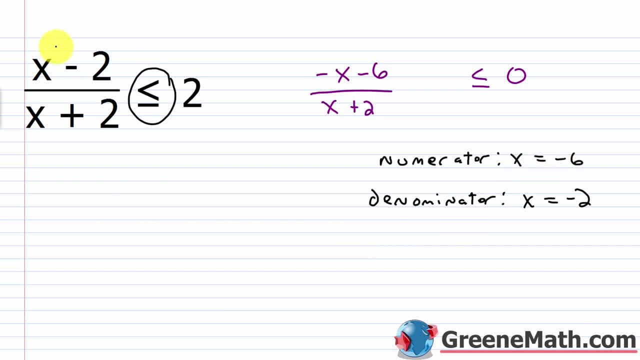 equal to. If I use x, equals negative 6, plug in a negative 6 here, So you get negative 6 minus 2.. That's going to give you a negative 6 minus 2.. So you have a negative 6 minus 2.. So you have a. 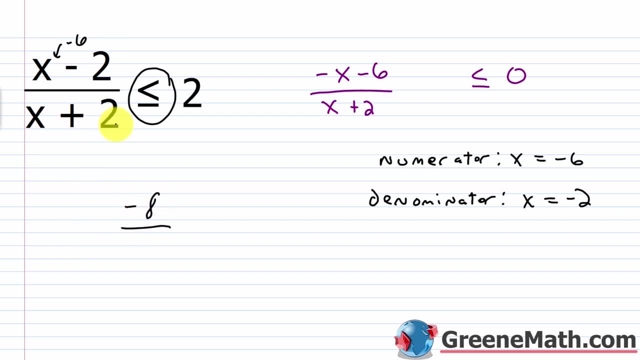 negative 8.. So you'd have negative 8 over. you'd have negative 6 plus 2, which would give me negative 4.. This is less than or equal to 2.. Negative 8 over negative 4 is 2.. So what you? 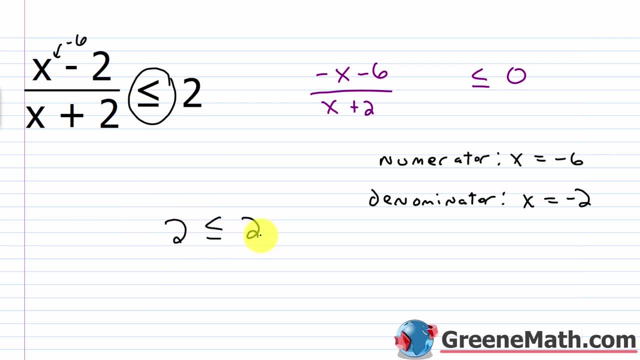 end up with. here is a true statement: 2 does equal 2.. So this part right here: x equals negative 6, this is going to work out for us. What's not going to work out for us is the denominator part where it says x equals negative 2.. This will not be a solution If I plug in a negative 2 for x. 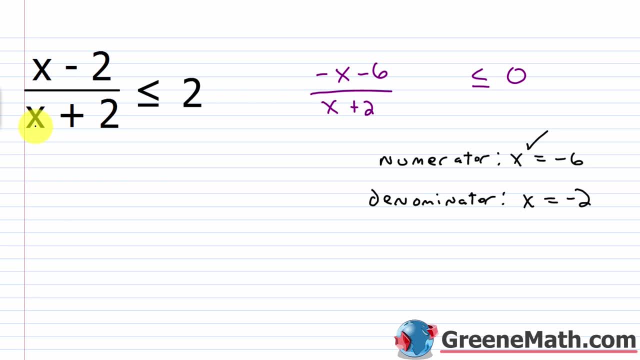 I'm going to get a zero denominator, So you've got to pay attention to those endpoints. you get One's going to work here, One's going to not. So let's get this down there. So again, x equals negative 6.. That's going to be right here, And I'll draw a little vertical line for 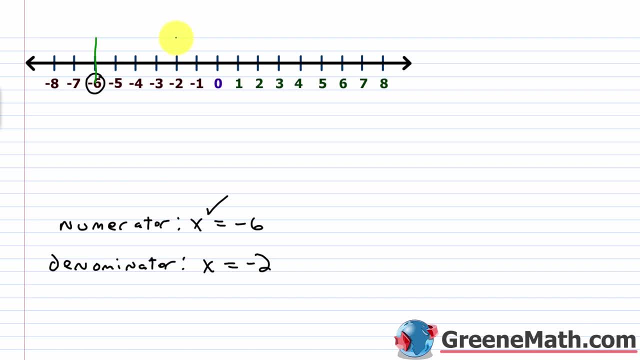 myself. And then x equals negative. 2 is right here. I'll draw a little vertical line for myself there. So let's call this region A, Let's call this region B, Let's call this region C. So in region A we can just choose negative 7.. 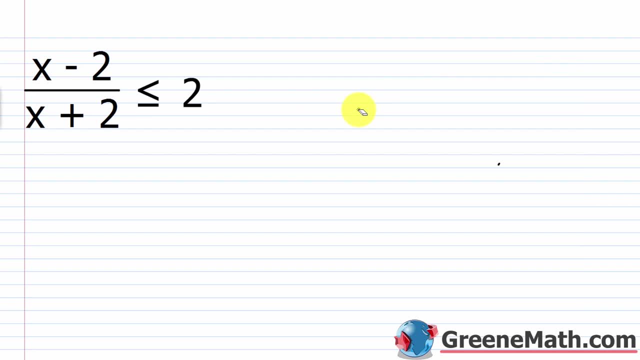 Let's erase this. And if I plugged in a negative 7 here and here, what would happen? Negative 7 minus 2 is negative 9.. Negative 7 plus 2 is negative 5.. Negative 9 over negative 5 is 9. 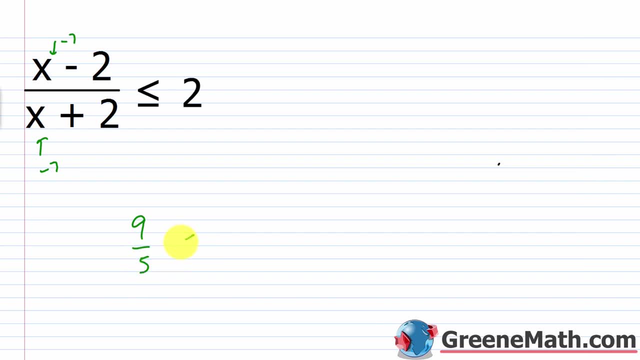 fifths, So 9 fifths. Is this less than or equal to 2?? Well, yes, it is. I would need a numerator of 10 to produce a result of 2, right 9, divided by 5.. 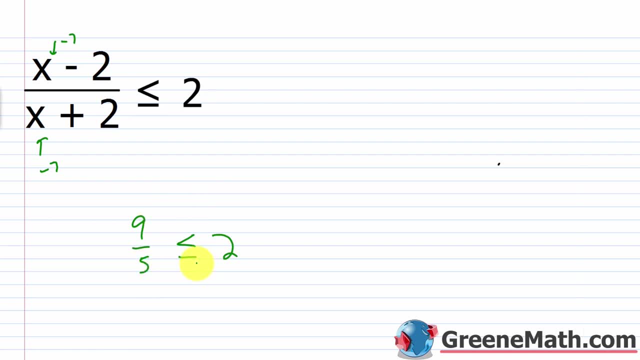 It's going to be less than 2.. So this satisfies the inequality. We could say: this is true. So anything in region A is true. What about region B? We could choose something like negative 4.. So for negative 4,. 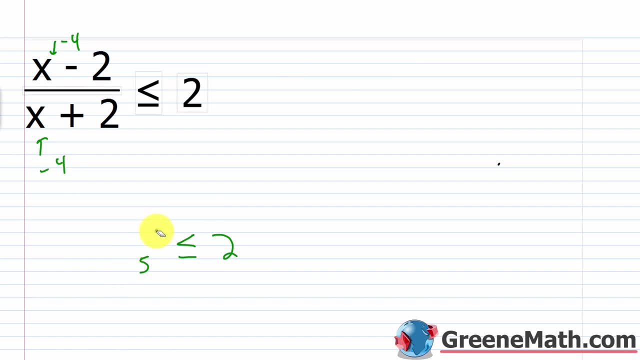 if I had negative 4 minus 2,, I get negative 6.. If I had negative 4 plus 2,, I get negative 2.. Negative 6 divided by negative 2 is positive 3. So you'd have: 3 is less than or equal to 3.. 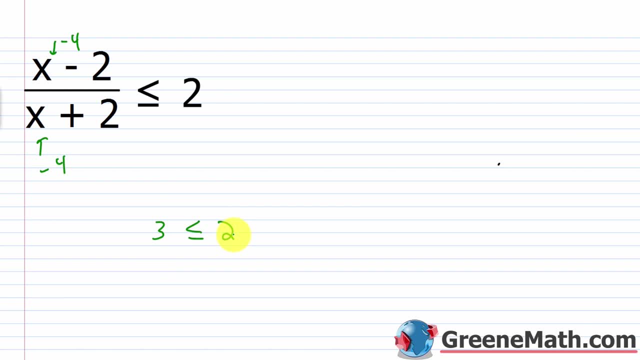 3 is not equal to 2.. That's false. 3 is not equal to 2.. And 3 is not less than 2. So that does not work. So anything in region B is going to be false. Then for region C I can choose 0.. So if 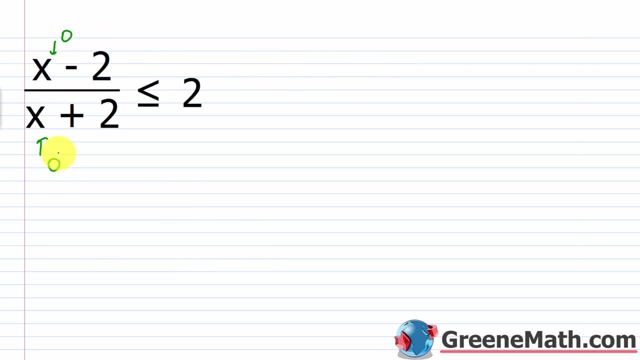 I plugged in a 0 for x. I would basically have negative 2 over positive 2, which would be negative 1. We would say negative 1 is less than or equal to 2. That's true. So for region C. 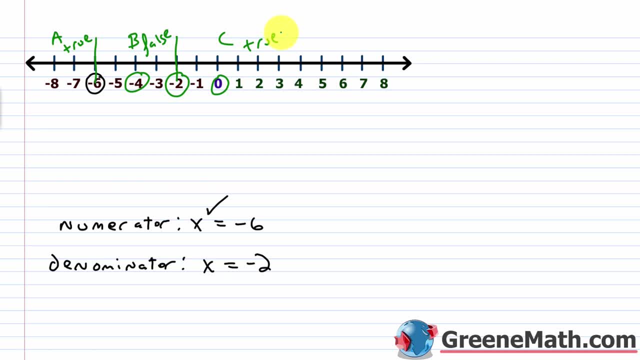 we would say this is true. Now, again, when we think about our solution, x equals negative 6, the one that came from our numerator is going to be part of our solution. So let me erase all this And I'll say: x equals negative, 6 is part of the solution. So I'll put. 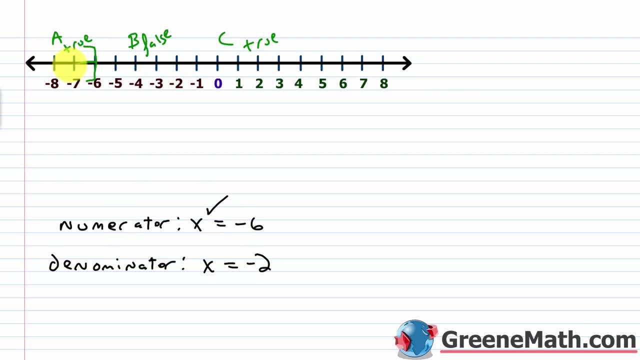 a bracket there And then anything to the left of that is going to work. Anything to the left Now at x equals negative 2, negative 2 is not going to be part of the solution That made the denominator 0. So I'm going to put a parenthesis there And then I'm going to 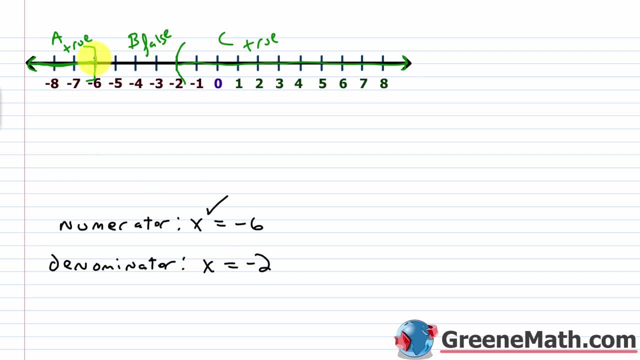 shade everything to the right. So anything that is negative 6 or less, and then also anything larger than negative 2 would work as a solution here. Let's erase this. And solution set notation, we'll say the set of all x, such that x is less than or equal to negative 6, or x is greater than. 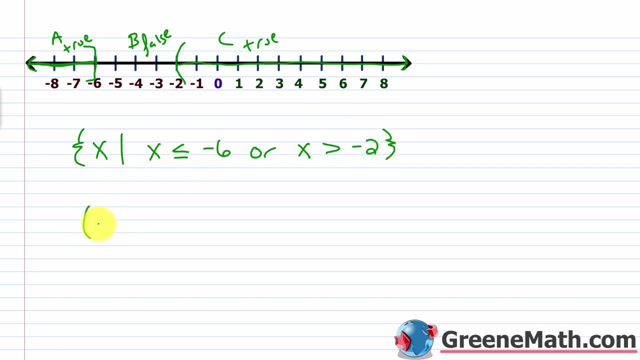 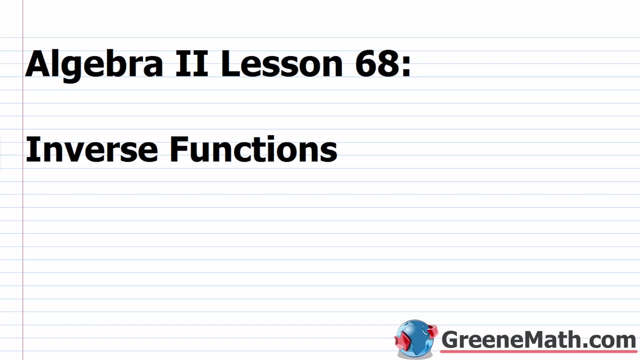 negative 2. And then an interval notation coming from negative infinity up to and including negative 6. So you get a bracket there and then the union width will have a parenthesis here, because negative two is not included out to positive infinity. Hello and welcome to Algebra 2, Lesson 68.. 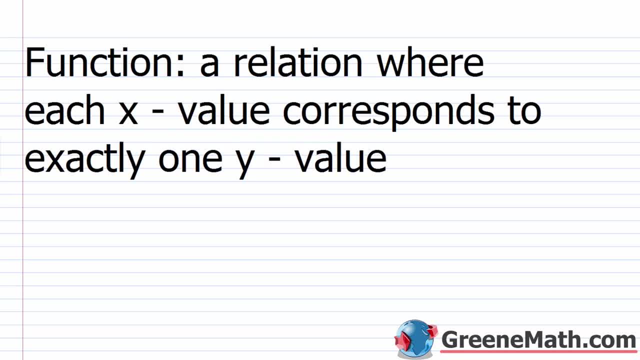 In this lesson we're gonna learn about inverse functions. So at some point in your Algebra 2 course you're gonna run into this topic known as inverse functions, And really this is going to lay the groundwork for us And we're gonna start talking about exponential functions. 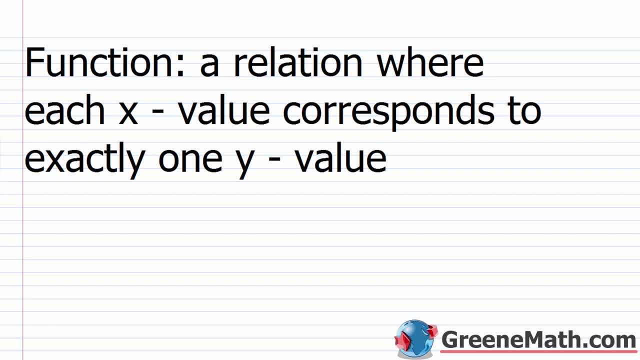 and logarithmic functions as soon as we conclude with inverse functions. So when we think about inverse functions, basically we're thinking about functions that reverse each other. But before we kind of jump in and start talking about inverse functions, I wanna just make sure that you understand. 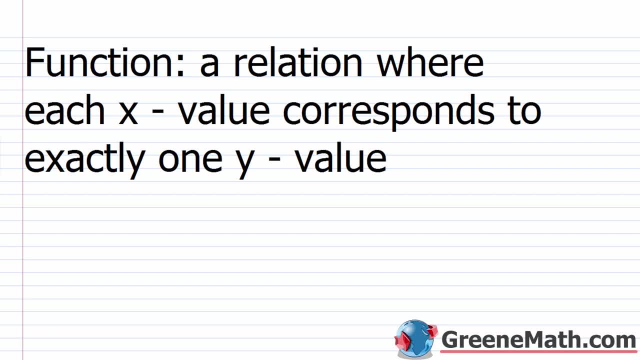 the basics of a function, So we wanna just do a quick review. At some point in either Algebra 1 or at the beginning of Algebra 2, you talked about functions and we learned that a function was nothing more than a relation or a set of ordered pairs. 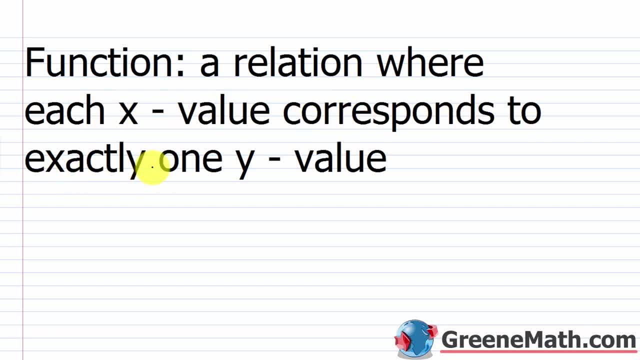 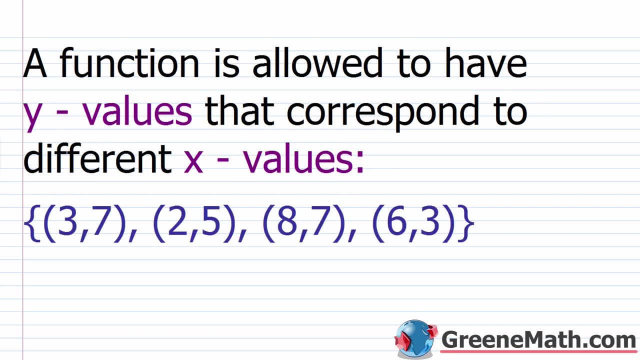 where each X value corresponds to exactly one Y value. So there's a clear association with a function. I give you an X value and you can tell me what the Y value is that's associated with it. So as an example, let's say we look at this set of ordered pairs here: 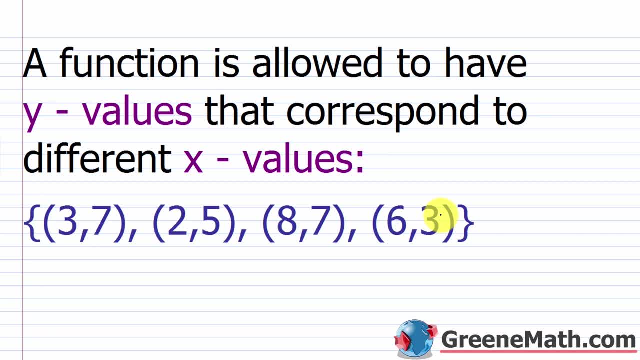 this relation and we say: is this a function? So for each X value is there a unique Y value that's associated with it. In other words, is there a clear association. So to see this, let's kind of draw a typical picture. 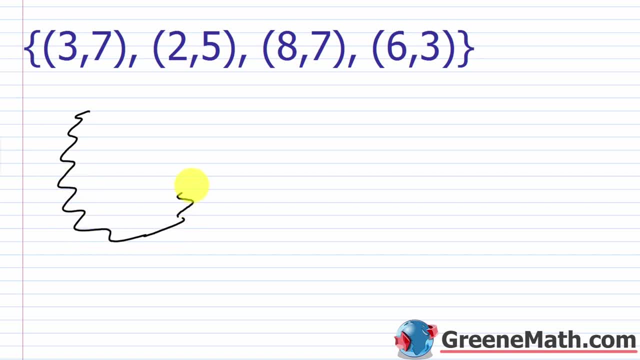 that you'd see in this section. So let's set this up and say that this is the domain. This is the domain, or again, the set of allowable X values. So what exists in our domain here? Well, we just have a set of ordered pairs. 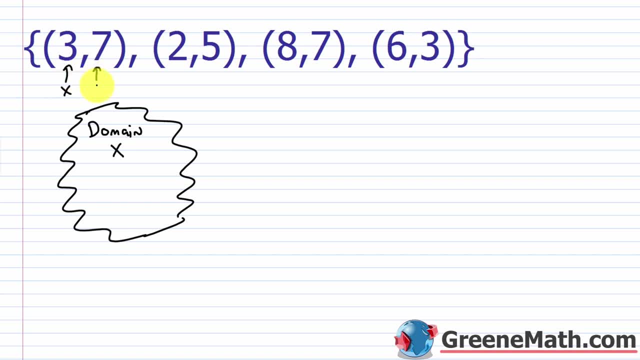 So, remember, the ordered pairs are X, comma, Y, So the first component or the first entry in each ordered pair represents the X value. So we have an X value of three, we have an X value of two, we have an X value of eight. 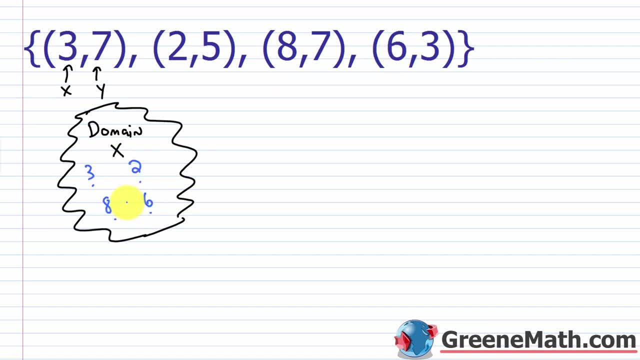 then we have an X value of six. So our domain consists of those four numbers. When we think about the range, okay, the range, that's the set of allowable Y values. So in this case our range consists of seven, five. 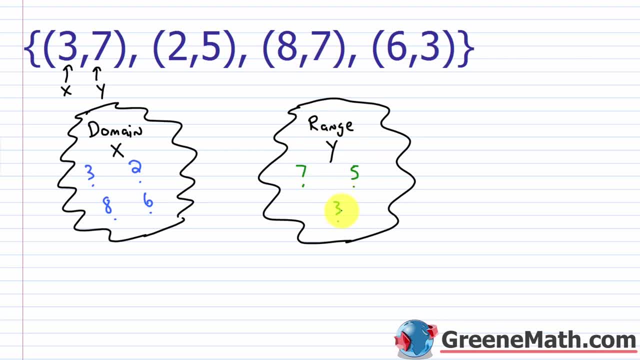 we have a seven again, so I'm not gonna double list that- and then three. Now again with a function. for every X there's gonna be a clear association with a Y value. So if I ask you, what is Y when X is three? 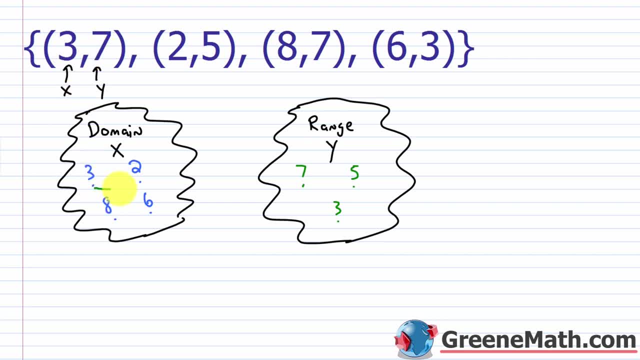 Well, when X is three, Y is seven. So there's a clear association there. When X is two, Y is five. So when X is two, Y is five. When X is eight, Y is seven. So when X is eight, Y is seven. 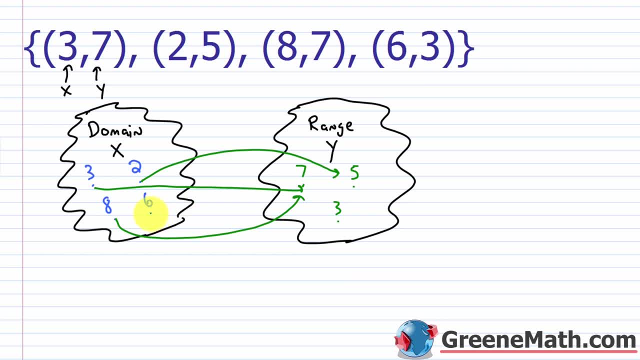 And then when X is six, Y is three. So when X is six, Y is three. So this is a function, because for every X value there is a clear association with one and only one Y value. Now the common thing that comes up in this section is that 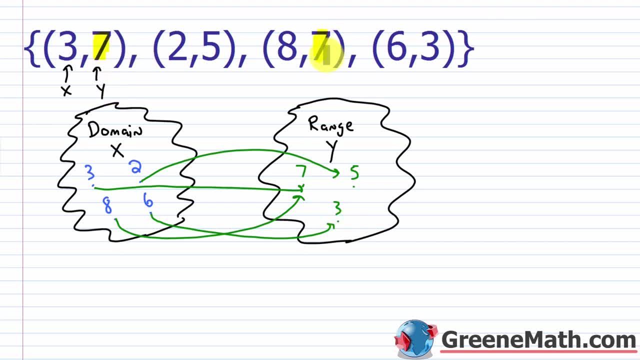 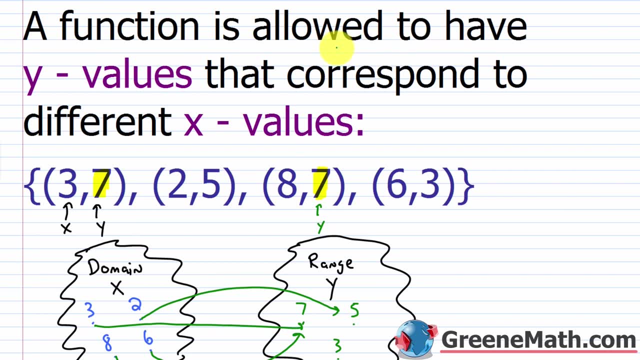 hey, well, I have a seven here for Y, and then I have a seven here for Y as well, And you'll see that I listed this up here. Here we said that a function is allowed to have y values that correspond to different. 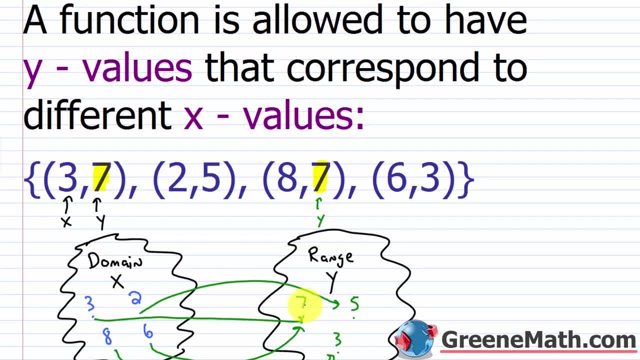 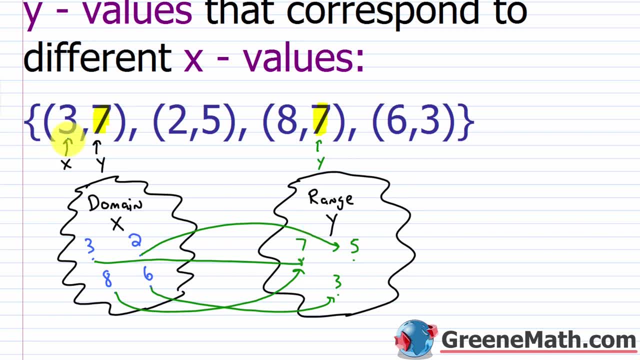 x values. So we have that here and that's allowed because, again, there's still a clear association. If I say, hey, x is 3, what's y? I know the answer is 7.. If I say, hey, x is 8, what's y? 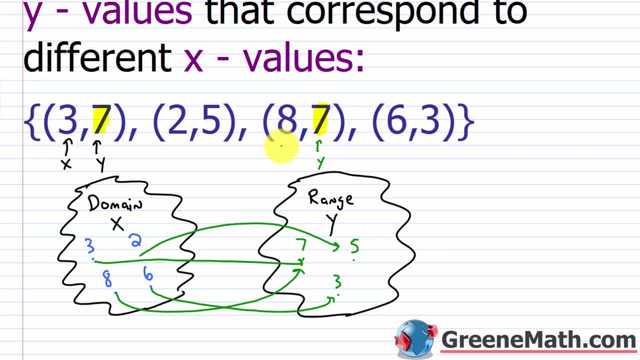 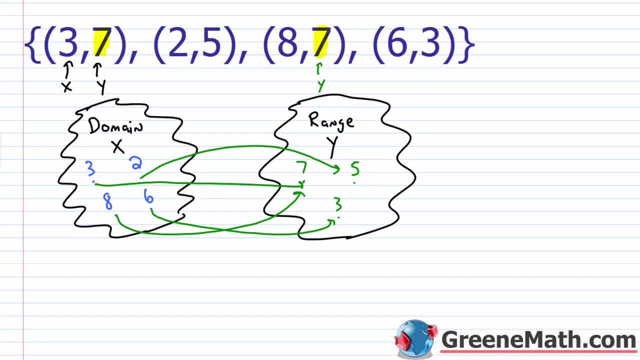 I know the answer is 7.. So it's okay that that occurs, because I have a clear association What I cannot have. let me kind of scroll back down with a function if I erase this and this and let's say I change this up a little bit and I say now I have the ordered. 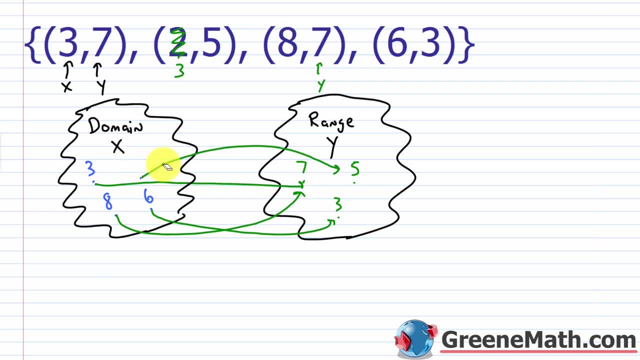 pair 3, comma 5.. So let's erase 2 from the domain and let's say that 3 is now mapped to or linked with 7, but 3 is also linked up with 5.. So the reason this violates the definition of a function is that x does not have a clear 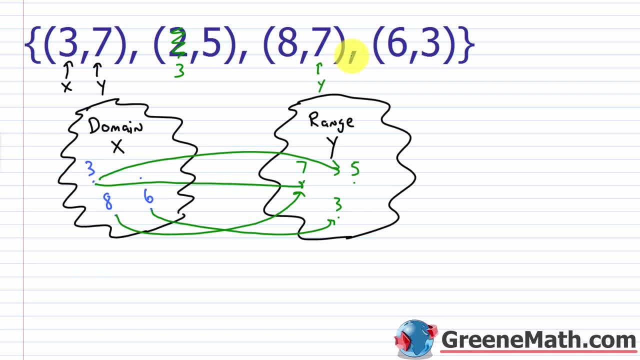 association with a y value. If I say, hey, if x is 3, what's y? You do not know whether to answer 7 or 5, right, Y could now be 7 or it could be 5.. So that's why we always say, for each x value, there is one and only one y value. 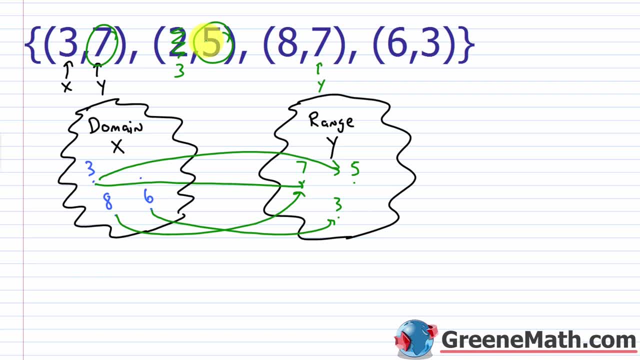 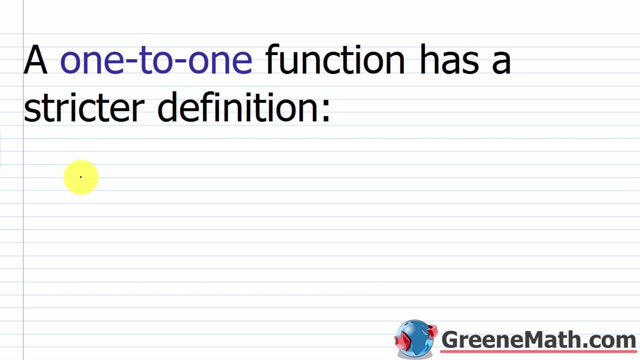 So there can be a y value that's associated with more than one x value, but there can't be an x value that's associated with or linked up to, more than one y value. Now we're going to introduce the concept of a y. We're going to use a one to one function, and you have to understand this to be able. 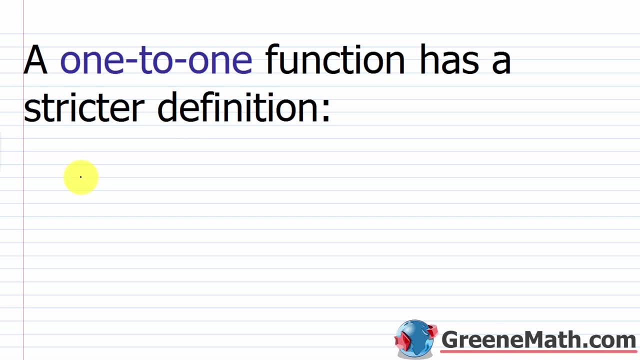 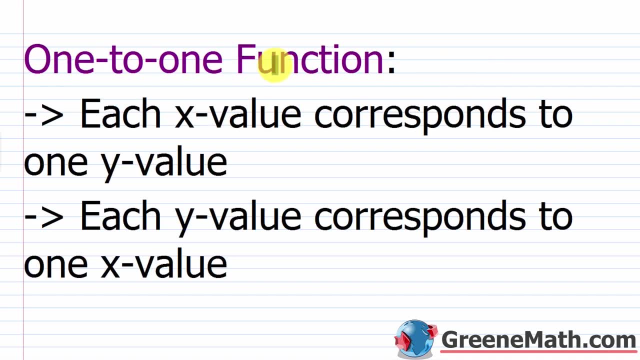 to get into this topic of inverse functions. So a one to one function, let me just highlight that, has a stricter definition. With a one to one function we see that each x value corresponds to one y value. That's the same as before. 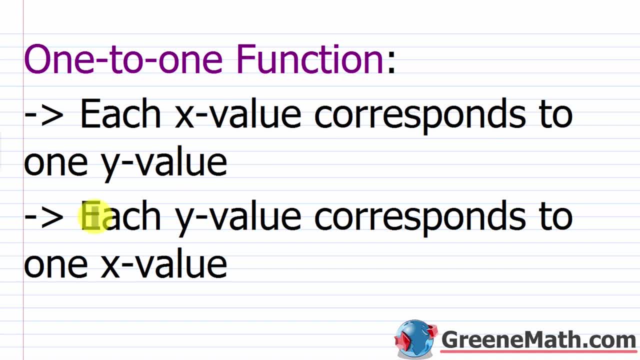 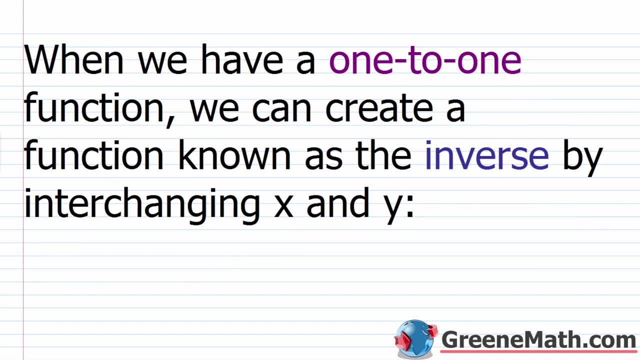 Okay, we've always had that rule, but now we're going to say each y value corresponds to one x value. Alright, so when we have a one to one function- and we'll learn how to determine if we have one or not later on in the lesson- but assuming that you do have one, we can create a function. 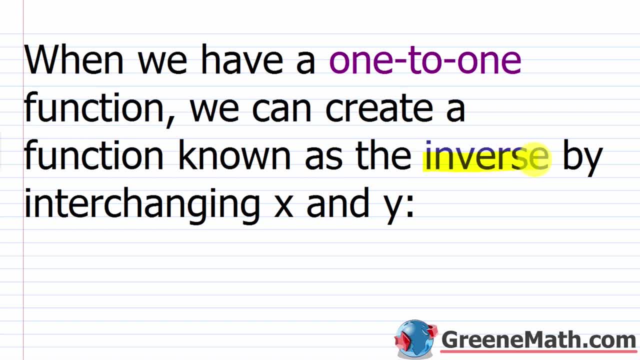 known as the inverse. okay, The inverse. and this is by interchanging, so in other words swapping x and y. So your x values become y values, your y values become x values. So we talk about the set of x values as the denominator. 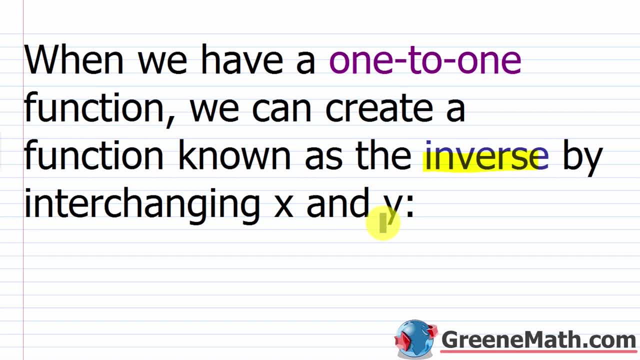 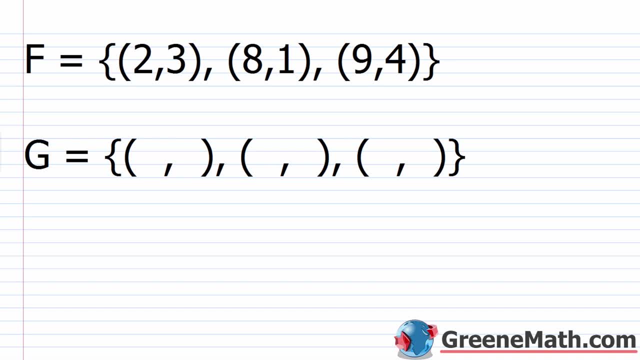 We talk about the set of y values as the range. So the domain of the original function will become the range of the inverse And the range of the original function will become the domain of the inverse. So if I have this function f and it consists of the following three ordered pairs: 2,, 3,. 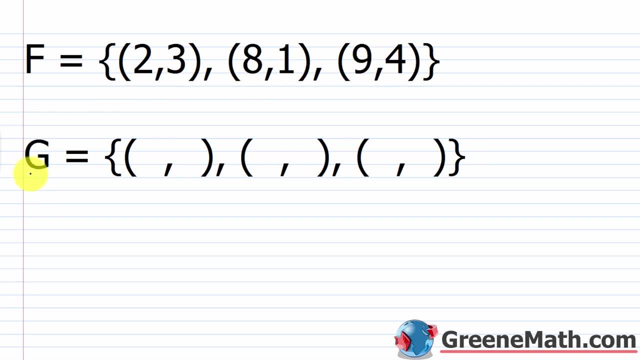 8, 1, and 9, 4.. And let's say we want to set this up to where g is the inverse of f. So these two, we're just going to interchange x and y. So if this is x and this is y, then I just want to interchange the two and say that this. 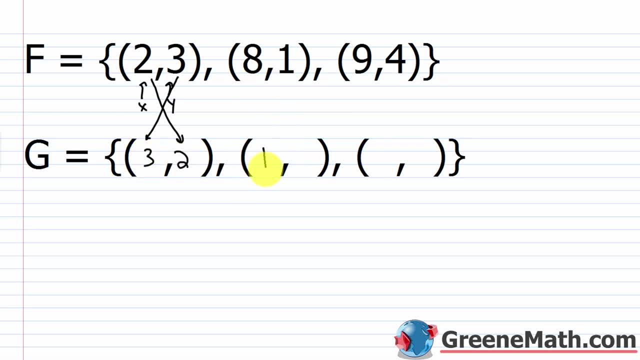 first ordered pair will be 3, 2.. The second will be 1, 8, and the third one will be 4, 9.. So the domain for f, the domain for f is what It consists of: 2, 8, and 9.. 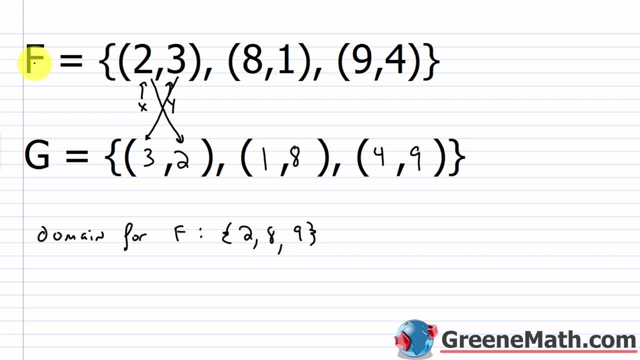 So those values are the x values in the original function, The original function f. Now we interchanged them when we created the inverse, which is g. So now the x values became y values. so when we think about the range, the range for g, 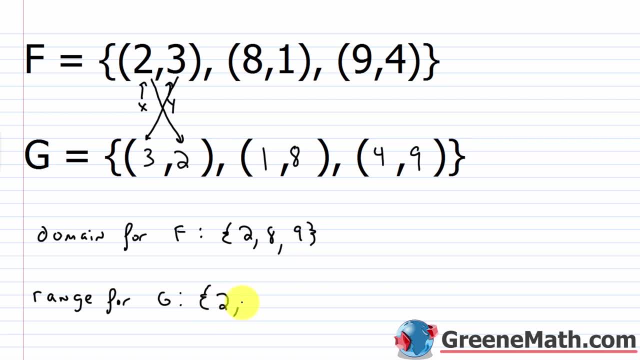 is what It's going to be, these values. So it's going to be 2,, 8, and 9.. And you can see that You have 2,, 8, and 9 in the y location for each ordered pair. 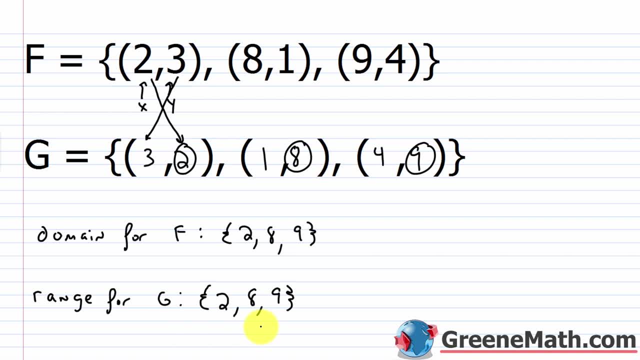 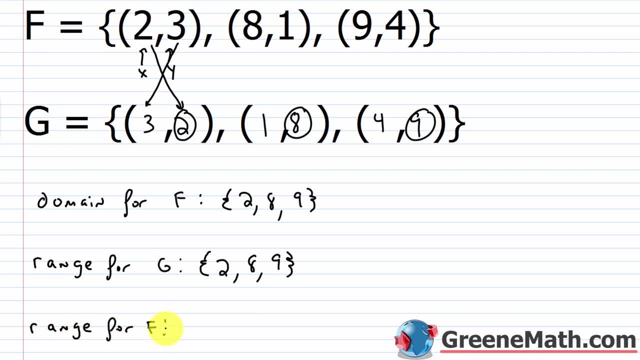 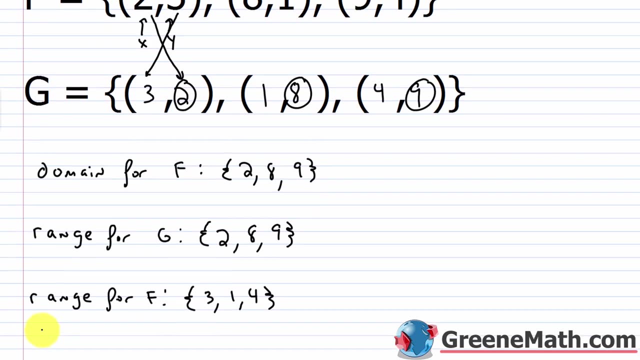 Right, So that's now your range When we think about the range for f. so the range for f, it's what It's: 3,, 1, and 4.. So 3,, 1, and 4.. 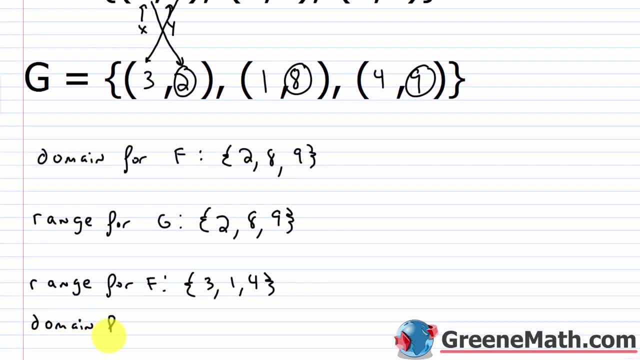 So then, when we think about the domain for g, it's going to be the range from f, Right, So it's going to be this right here. So 3,, 1, and 4.. So you see, you have 3,, 1, and 4.. 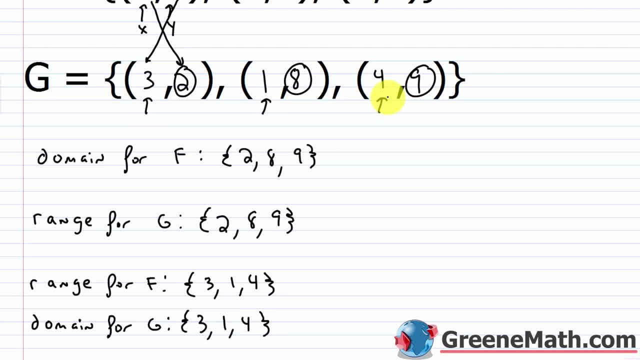 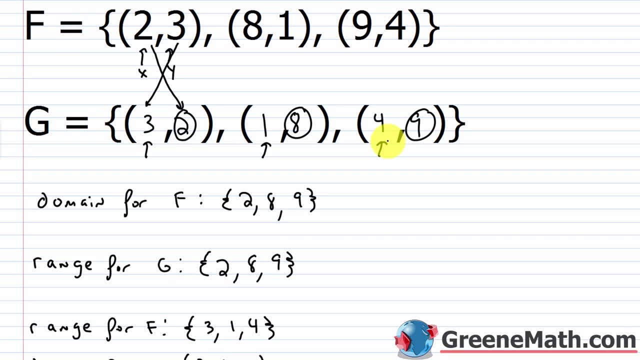 So you see you have 3,, 1, and 4 in your x positions there. So just a little simple example here for you to see what we mean by inverse functions and how the x and the y values are interchanged. So first we start out with f. 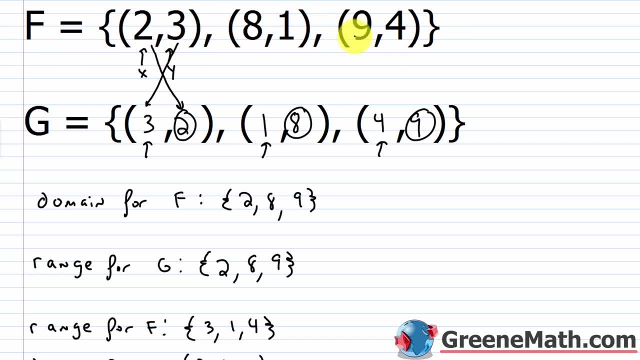 Again, this is a one-to-one function. You have x values of 2,, 8, and 9.. So nothing's duplicated there. Then you have y values of 3,, 1, and 4.. Nothing duplicated there. 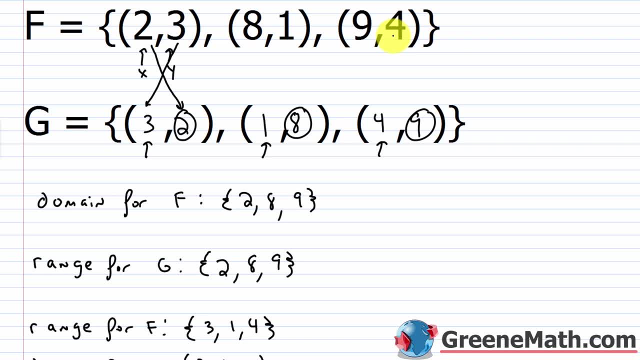 So when that occurs, for each x there's one y and for each y there's one x, So it's one-to-one Right. So then we can create this inverse, which is g, by just interchanging x and y. 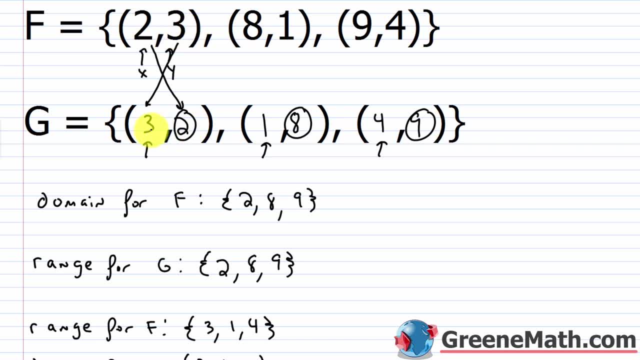 So we have the ordered pair 2, 3.. We swapped everything, So this became 3, 2.. So now 3 is the x value, 2 is the y value. Then we saw we went from 8, 1 to 1, 8, and from 9, 4 to 4, 9.. 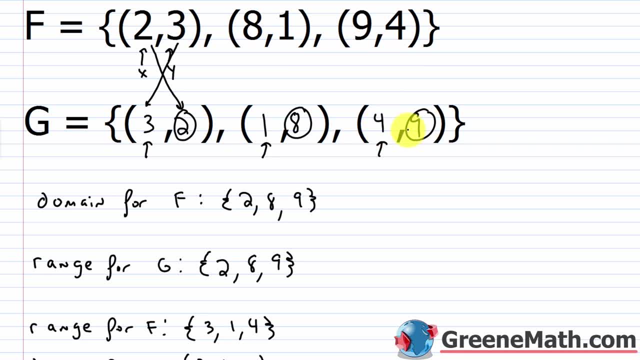 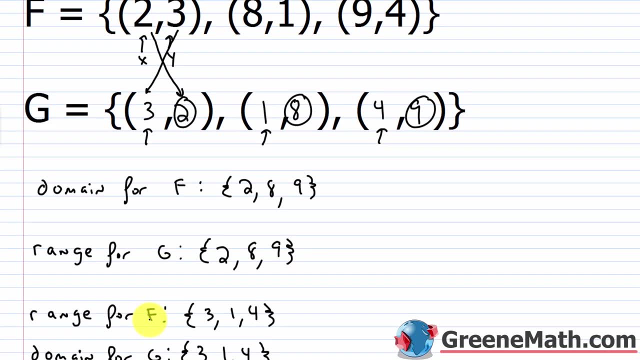 So obviously the domain or the set of allowable x values for f became the range for g, because we swapped x and y values, And then the range for f became the domain for g, Right Again, because we just swapped x and y values. 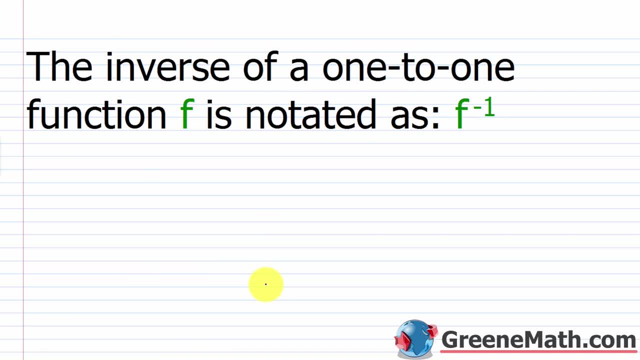 So the next thing we want to talk about is the notation that's involved with an inverse function. So this is a very big source of confusion for students. So the inverse of a one-to-one function, f, is notated as f inverse, So that's how that's read. 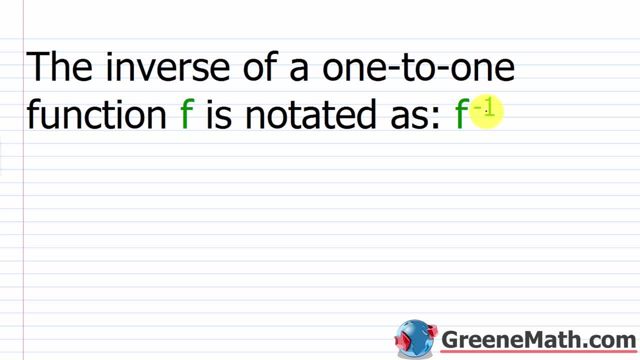 It's not f to the power of negative 1, like it appears to be. So this is a big source of confusion. If I have a function f of x, then I'm going to have a function f of x, And it's a one-to-one function. 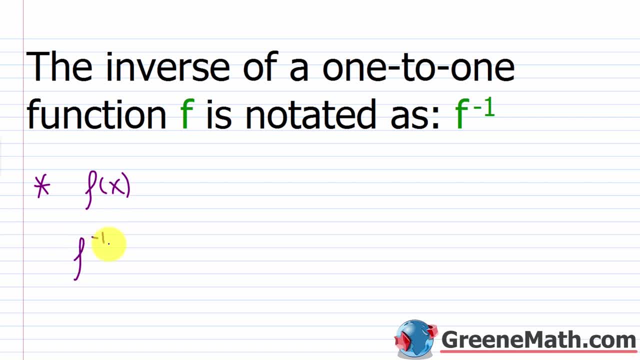 When I notate the inverse, I say f inverse, like that. That's what it means. So f inverse of x. So these two are inverses of each other. So these are inverses And basically that just means these two functions will reverse each other. 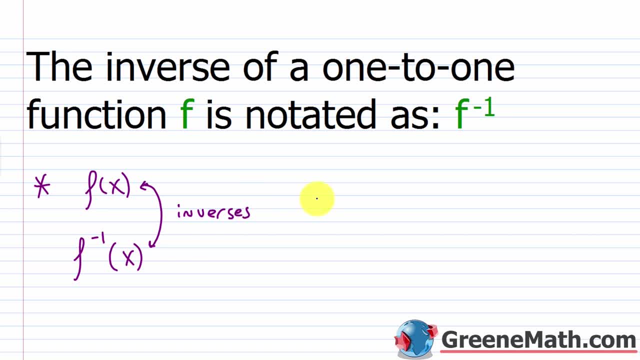 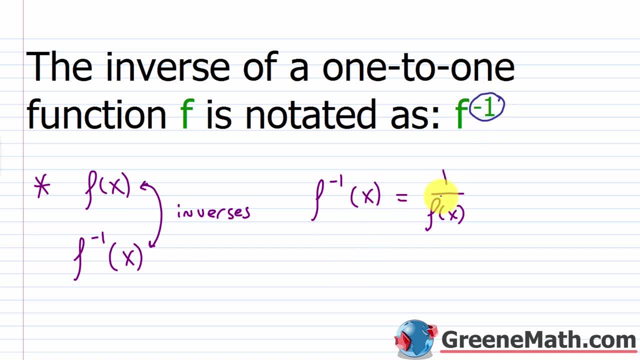 This is a common mistake, Again, because you see that negative 1 there you're thinking about the rules of exponents. This is wrong, OK, Wrong, And again, I don't know who set this up, But it's really, really confusing when you look at the notation. 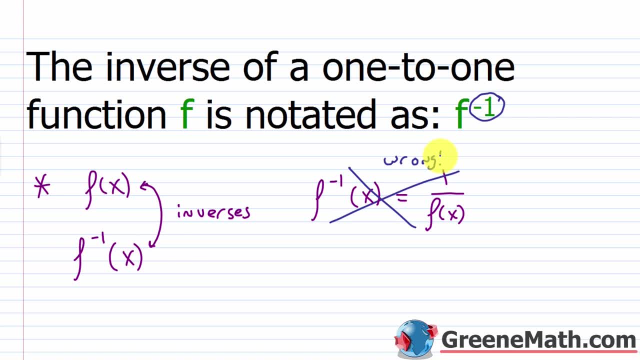 especially if you don't have somebody there to tell you. If you just read it in a book and they don't tell you that, you might really think that This is f to the power of negative 1, right, It's not. 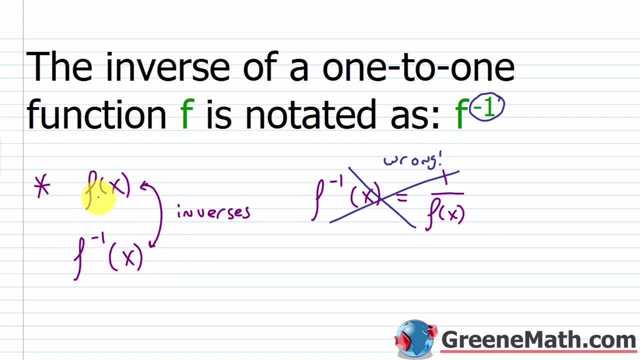 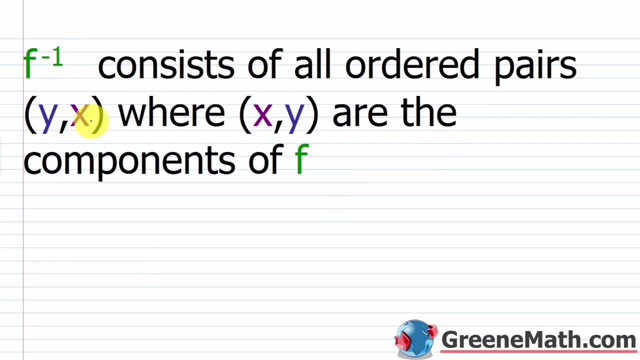 So this is f inverse of x. Again, that's the inverse of f of x. All right, So f inverse consists of all ordered pairs, y comma x, where x comma y are components of f. So we saw that with the simple example. 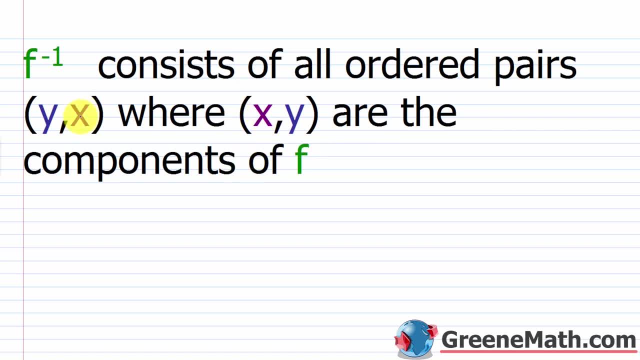 We saw that every x value became a y value in the inverse. So if this is the original right here, my x value here goes Into the y position And then my y value here goes into my x position. So the x values become y values. 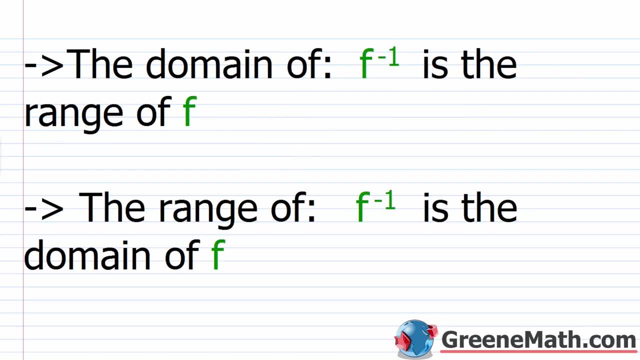 The y values become x values, And we talked about this already. The domain of f inverse is the range of f. So in other words, the x values of the inverse came from the y values of the original And then the range or the y values of the inverse. 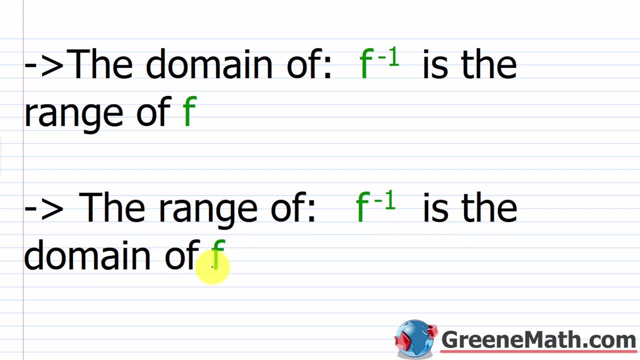 is the domain of f, So the y values of the inverse Came from the x values of the original function. So I know this looks a little complicated in this form, But when you break it down like that it's super simple. x values of the original function become y values. 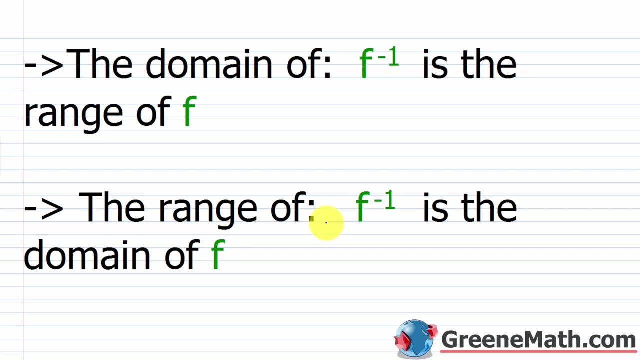 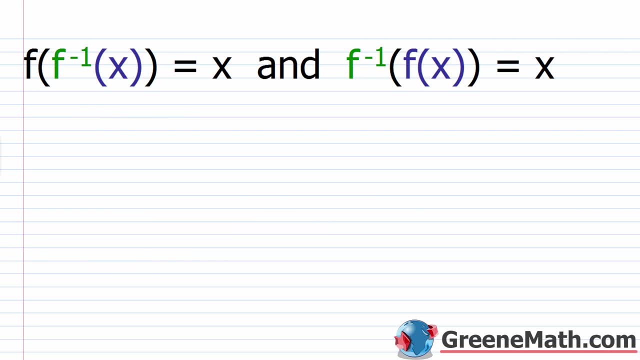 of the inverse, And y values of the original function become x values of the inverse. All right, So you might see this notation in your textbook when you first get started, And a lot of students get really confused with this one too. So I just want to take a moment and kind of break this down. 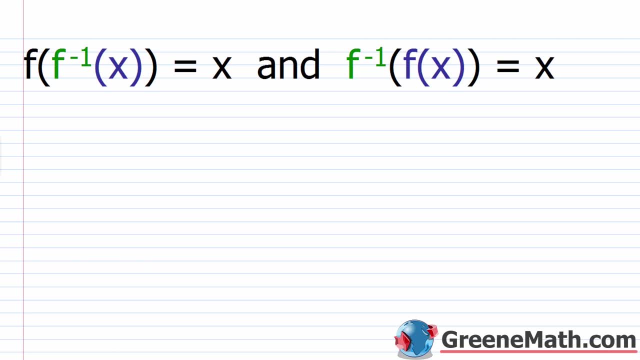 I want you to see an example where you can look and understand How the functions reverse each other when they're inverses. OK, So if we see f of f inverse of x, we say this is equal to x. We also see that f inverse of f of x is equal to x. 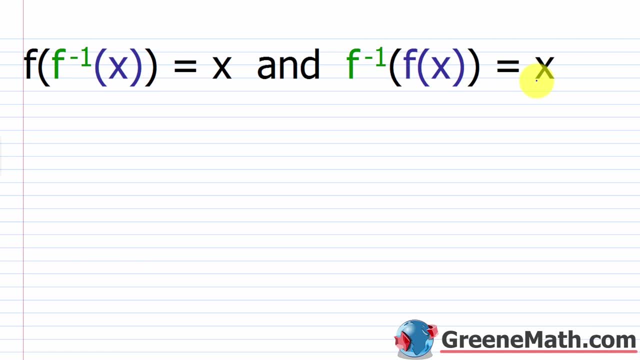 So you might say: what in the world does that notation mean? So let's look at an example And then we'll kind of work through that, And then we'll come back in the end And we'll explain what this generic notation means. 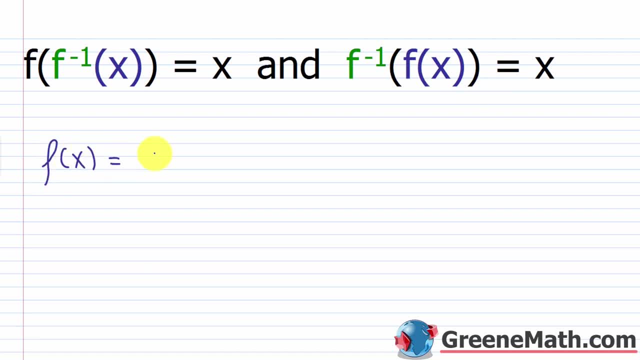 Let's say you had f of x is equal to 2x plus 3.. OK, Now I haven't taught you yet how to determine if something is 1 to 1.. We'll get to that later on in the lesson. 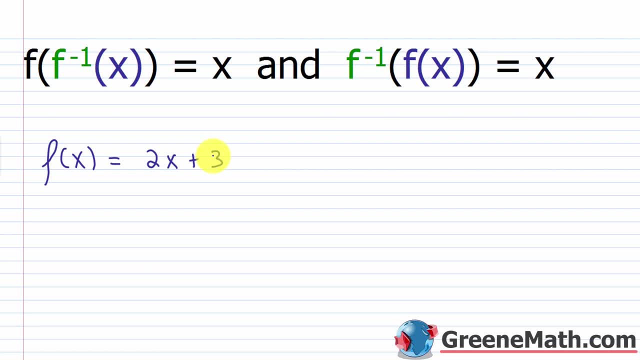 But I just want you to believe me when I say it is a 1 to 1 function And therefore it will have an inverse. Now how do we find the inverse? We'll talk more about this later, But the simplest method to do this: 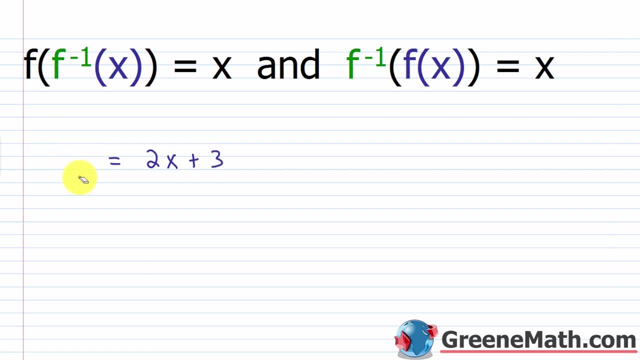 is to replace f of x with y. So we know, f of x just took the place of y when we started talking about functions. Why? Why? Because y or f of x is nothing more than the dependent variable. That's all it is. 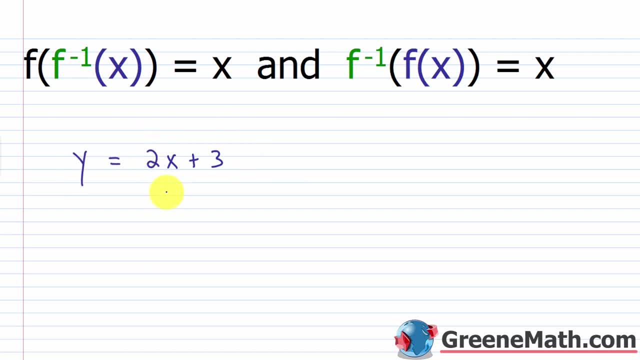 So y is equal to, or y is the same as this quantity, 2x plus 3.. OK, Now all we need to do is swap x and y, So y becomes x And x becomes y. All right, So now we're going to solve for y again. 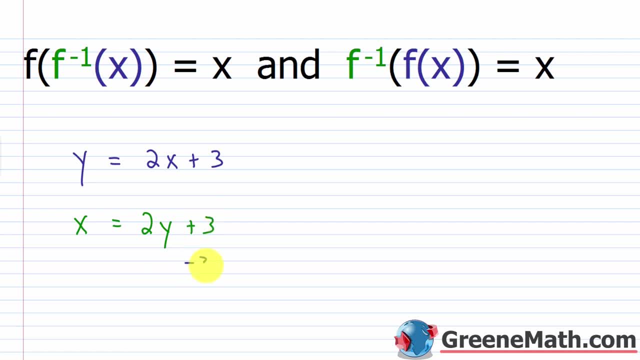 So to do that, I would subtract 3 away from each side of this equation And that would give me what I would have. x minus 3 on the left is equal to. This would cancel, So just 2y. And if I wanted to solve for y, I 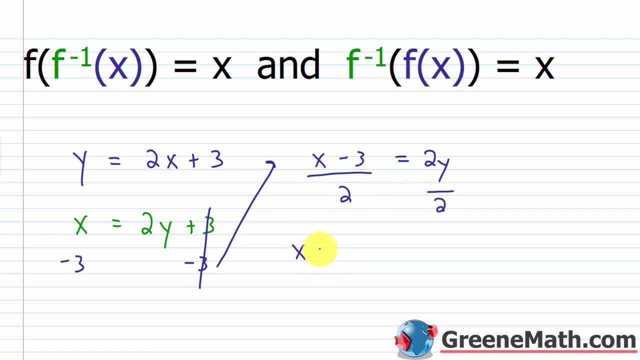 would divide both sides of the equation by 2. And I would have x minus 3 over. 2 is equal to y. This would cancel with this. Let's write this over here, So you have your original function, which is y equals 2x plus 3.. 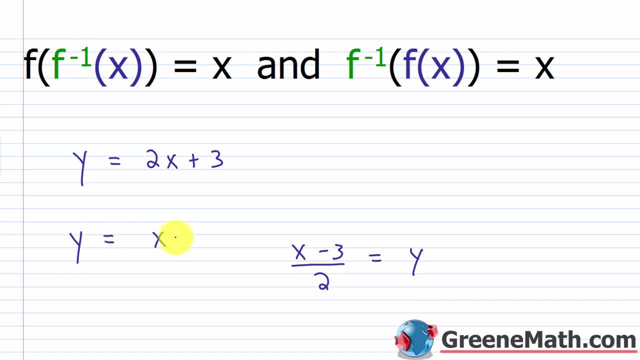 And then you have your inverse, which is y equals x minus 3 over 2.. So these two functions are going to reverse each other. Now the notation for this, remember, y is nothing more than f of x when we're talking about a function, and if these two are, 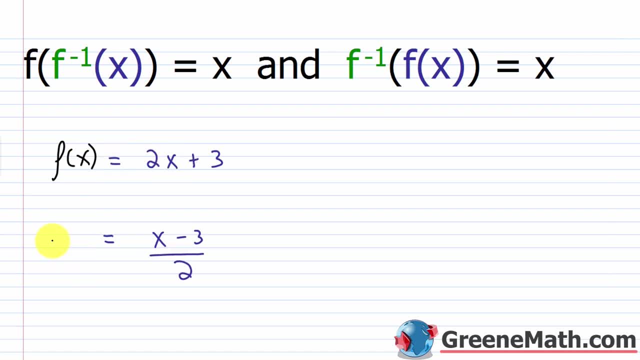 inverses, and this is the original. this is the inverse. so we notate it by saying f inverse of x. okay, very, very simple, All right. so now we have our two inverse functions. we have f of x equals 2x plus 3, and we have f inverse of x equals x minus 3 over 2.. So let me give you a little bit. 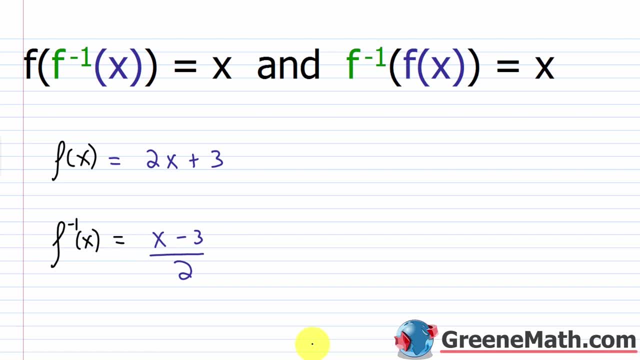 of insight right now into how these two functions are considered inverses of each other, or in other words, how they reverse each other. So if I start out with the original function, f of x equals 2x plus 3, I take x- whatever value I choose for that doesn't matter what it is- I multiply it by 2 to. 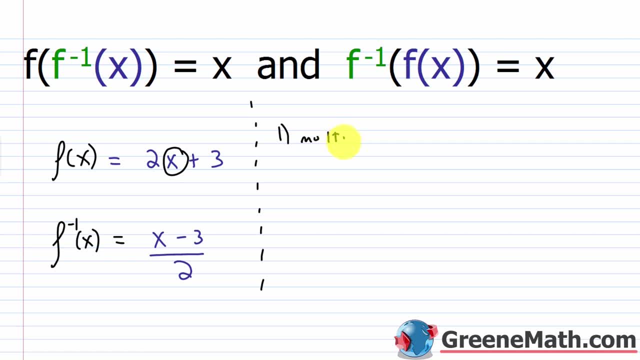 start. So kind of step one: I multiply x, x, x, x, x by 2.. Then in step two, once that's done, I'm going to add 3, so I'm going to add 3.. So as an example, let's say I choose 4 for x. So the notation for that with a function is f of 4, just means I'm. 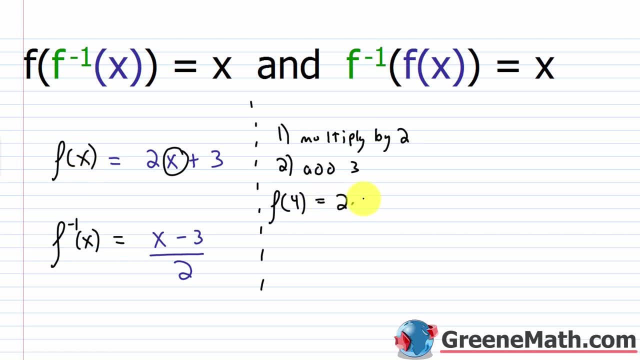 plugging in a 4 for x. So this equals 2 times 4 plus 3.. 2 times 4 is 8.. 8 plus 3 is 11.. Okay, let's think for a second what happens with the inverse So f, inverse of x. we first subtract the. 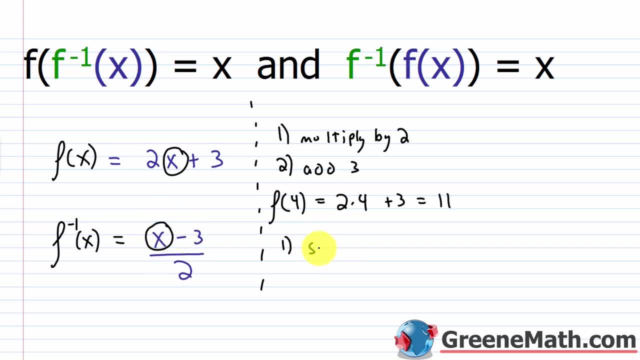 way 3 from whatever x is. So step one: we subtract away 3.. Now we can see that subtracting away 3 would undo the addition of 3 that we saw in the original function. Then, for step two, we see that once this numerator is done right- we subtracted away 3- we're going to divide by 2.. So we're going. 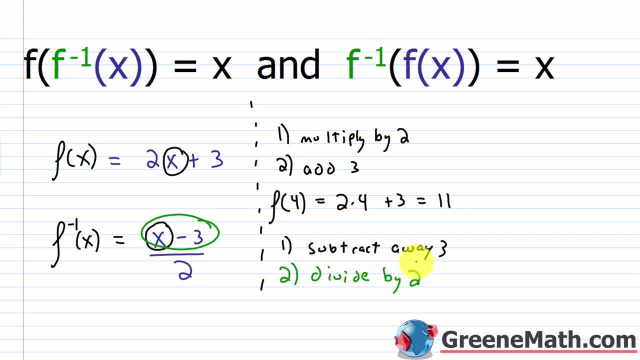 to divide by 2 and that undoes the multiplication by 2 that we did in the original step of the first function. So you can see how these two would reverse each other. So if I took f inverse of 11 of 11, I would reverse the process. 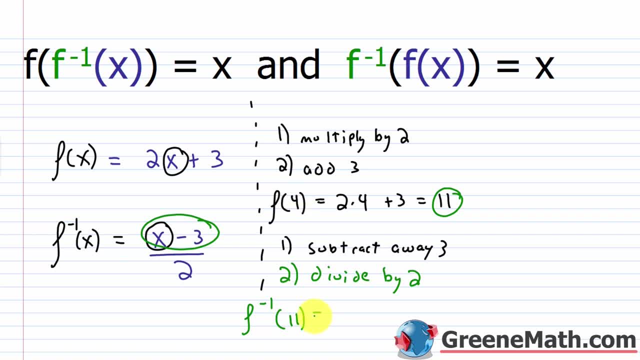 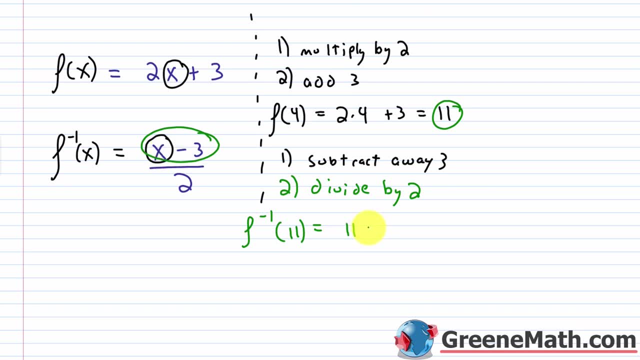 and I should get back to 4.. So this would be equal to what? So let me kind of scroll down a little bit, get some room going. This would be: plug in: 11 for x minus 3 over 2.. 11 minus 3 is 8.. So this would be. 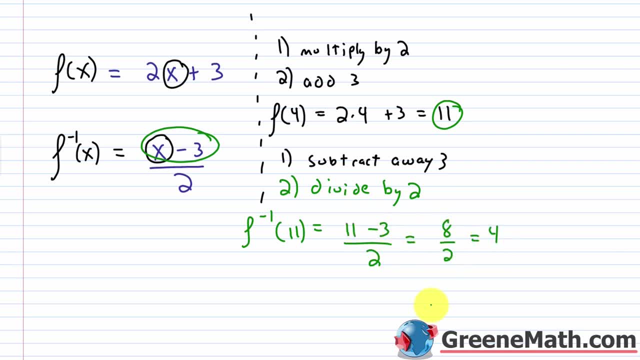 8.. So you'd have 8 over 2, which would give me 4.. So you can see how the x value of 4 became the y value of 4 in the inverse, And the y value of 11 became the x value of 11 in the inverse. So in other words, 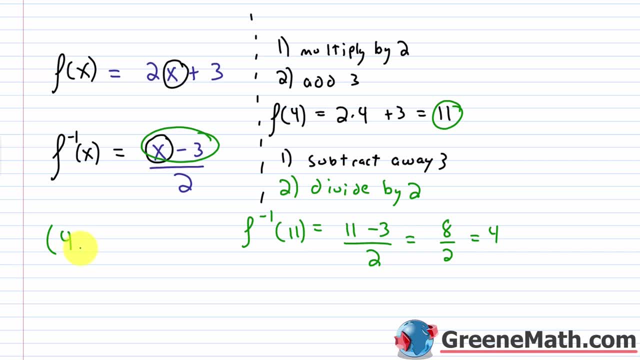 in the original function we have the ordered pair 4, comma 11.. Meaning I plug in a 4 for x and I get an 11 for y or for f of x. In the inverse function these two are interchanged. So in other words, I plug in 11 for x and I get a 4 for y. So you can see here. 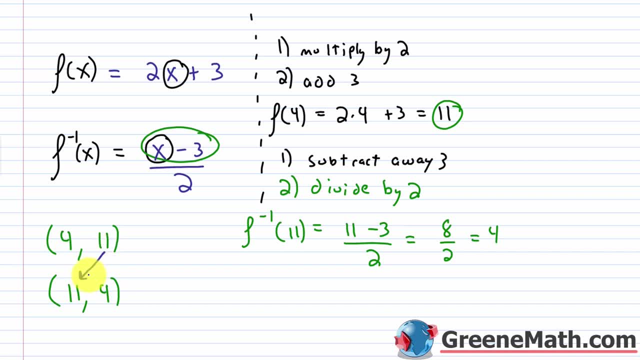 11 started out as y became x. 4 started out as x became y. So we're just interchanging the x and the y values. Now let me erase this and I'll show you this generically, and then we'll kind of move. 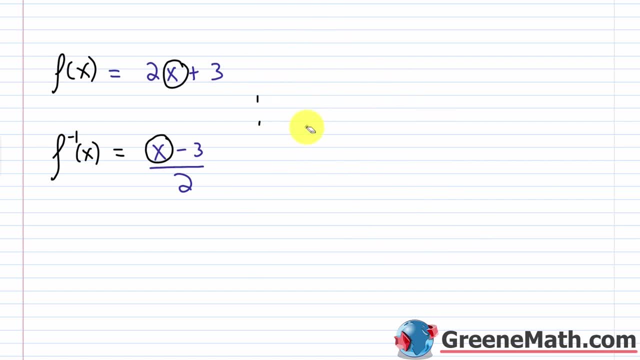 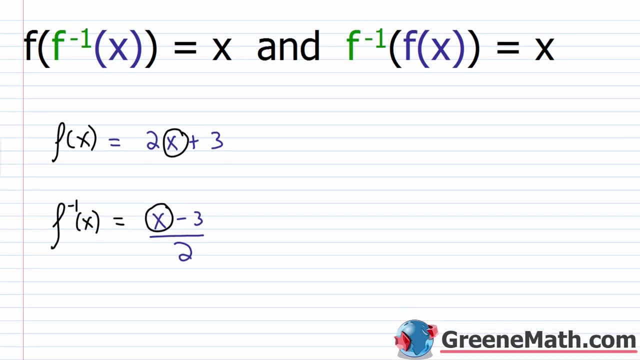 on to some other topics and we'll swing back to this. Let's scroll up a little bit and let's see if we can make sense of this notation here. So the first thing is that we have f of f inverse of x. What does that mean when we say f inverse? 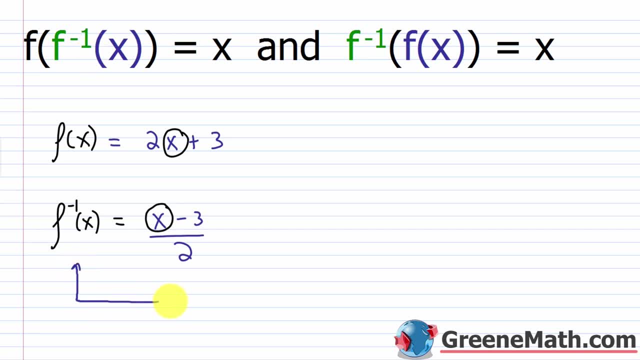 of x. So remember, when we think about an equation, the two sides are equal to each other, meaning they're the same as. So you might as well think of this. forget about the fact that it's an inverse. for a second, We can really just say: this is a function or an equation. 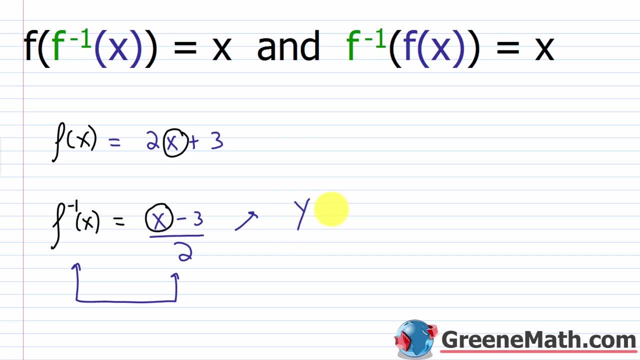 We say we have some dependent variable, let's just call it: y is equal to x, the independent variable, minus 3 over 2.. So if this right here is just asking me for what is y in the inverse, Well, y equals this guy right here. So I could plug that in right here. I could plug that in right here and 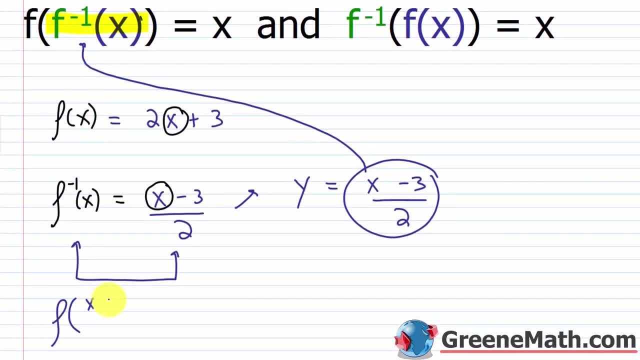 I could say in the original function: so f of x minus 3 over 2 should be equal to x. Let's see if that's the case. So this is equal to 2 times. I'm plugging this in for x. So I'm plugging. 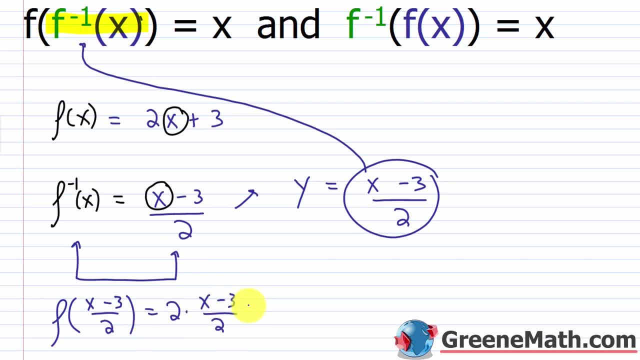 in an x minus 3 over 2 and then plus 3.. So what happens here is that this 2 cancels with this 2 and I'd be left with what I'd have: x minus 3 plus 3 minus 3 plus 3.. Those two cancel, I'm left. 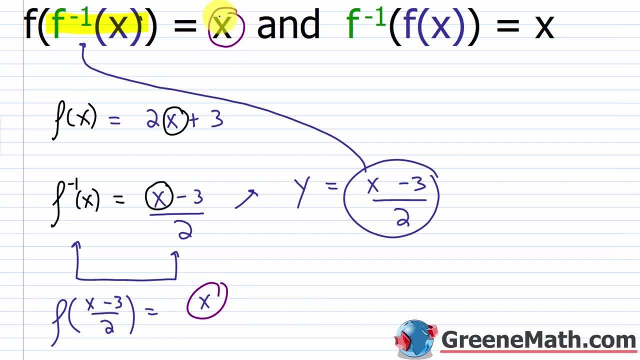 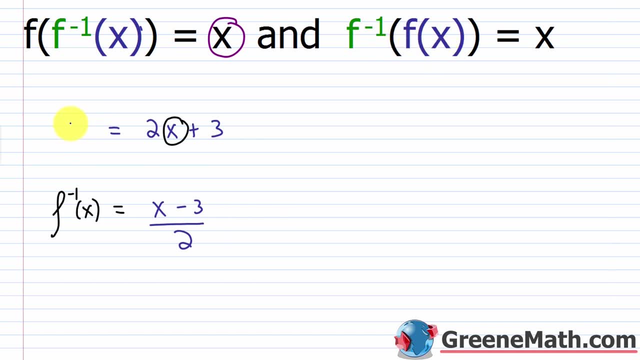 with x, which is exactly what it tells me I would be left with. If I think about f, inverse of f of x, f of x, or again, you could just think about this as y. if it's giving you a mental roadblock, this is equal to 2x plus 3 or it's the same as 2x plus 3.. So I could just plug this in here. I'm saying, hey, 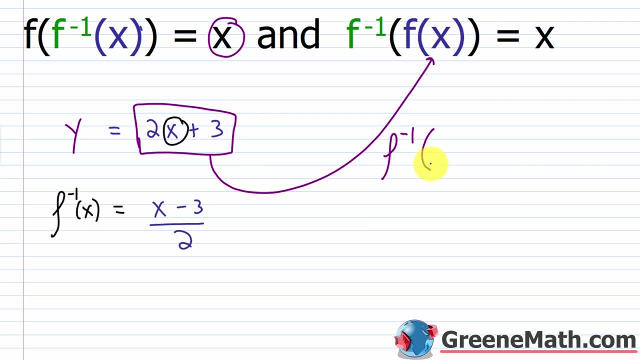 if I have the inverse function and I plug in the y from the original function, I should get x back. right? That's what I would expect, because if I take the y from the original function and I plug it in, I know I'm going to get x. So this is f inverse of, we'll say 2x plus 3, and this should. 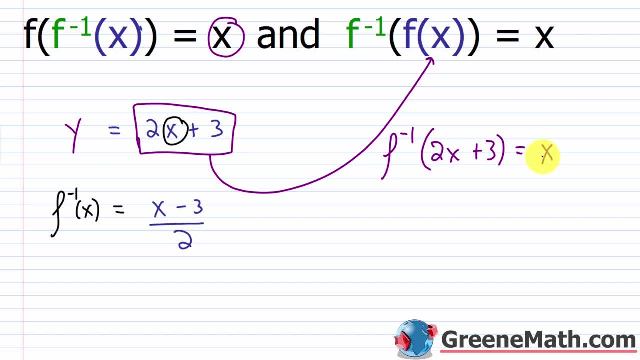 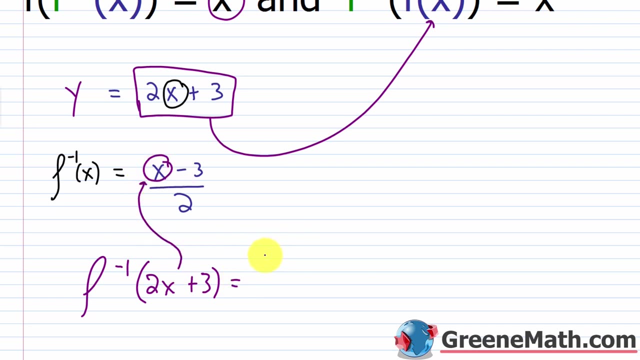 give me x back. Does that happen? Well, let's go ahead and calculate this. So let me kind of scooch this down and let's see what this gives us. So we would plug in a 2x plus 3 there, So we would have: 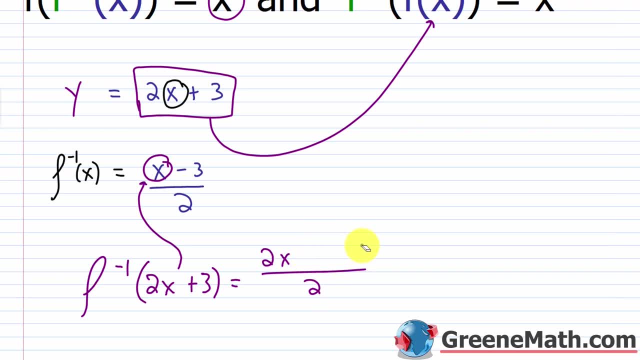 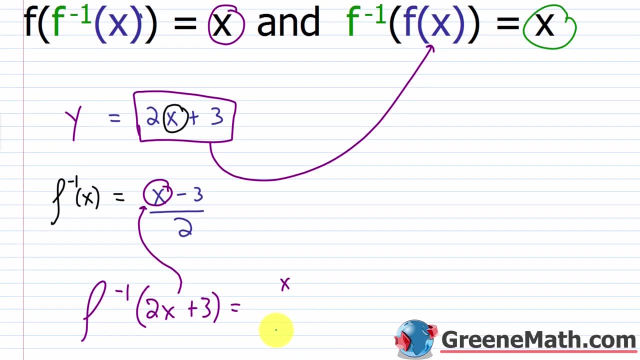 we know 3 minus 3 would give us 0. So this would basically be 2x over 2.. The 2s would cancel and again I'm just left with x. So hopefully this kind of clarifies some things for you. I know a lot of. 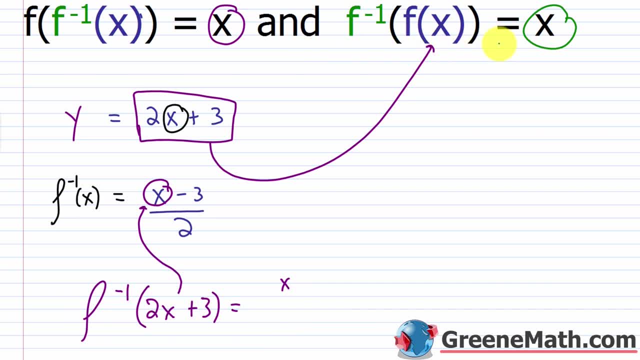 students will see this notation, just really freak out and say: what does it mean? Again, it all goes to this concept where the x and the y values are just interchanged. So the x values from one function will become y values in the other and the y values in one function will become x values in. 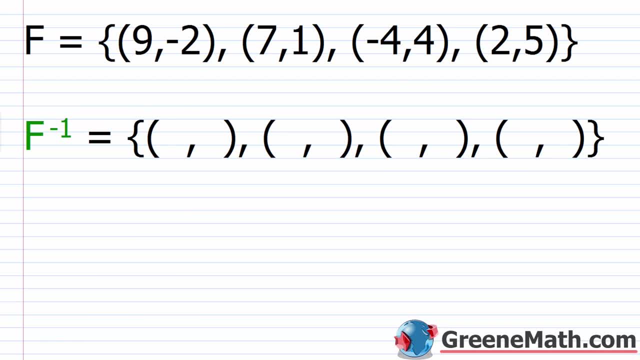 the other. All right, so let's kind of roll through this and see what happens. So let's go ahead and some problems now, and I'm going to talk to you a little bit about how to determine if something is a one-to-one function. So first let's look at this simple example. We have f here and we see that we 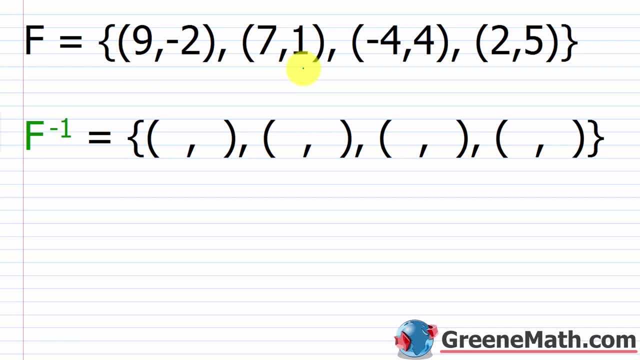 have 9 comma negative 2.. So this is our first order pair, then 7 comma 1, then negative 4 comma 4, then 2 comma 5.. We then see we want f inverse. So the first question would be: is this a one-to-one? 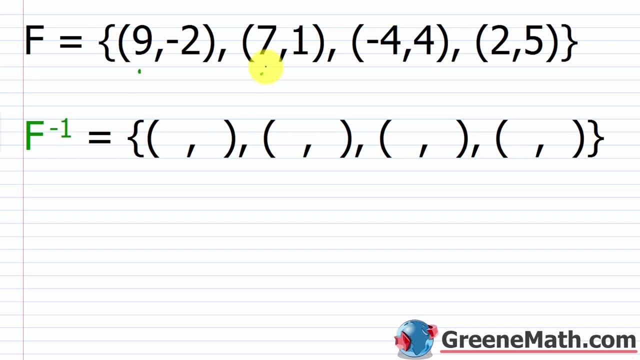 function I see for my x values I have 9,, 7,, negative 4, and 2.. So what's your question? So if you're actually looking for in a problem like this, you don't want any duplicate x values, because that would mean the same x value is linked up to more than one y value. Then you want to look. 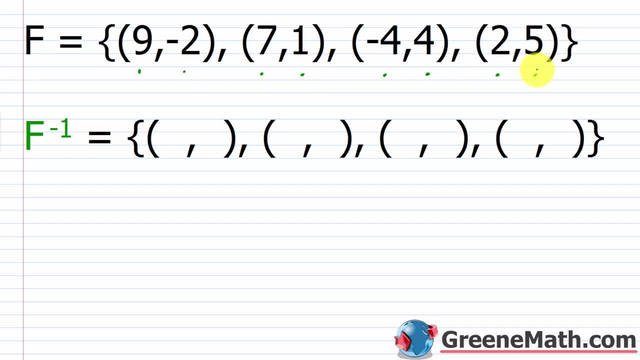 for duplicate y values. So negative. 2,, 1,, 4, and 5 don't have that. So you're looking for that to say: hey, each y value is only linked up to one x value, So this function is one-to-one, so it will have an. 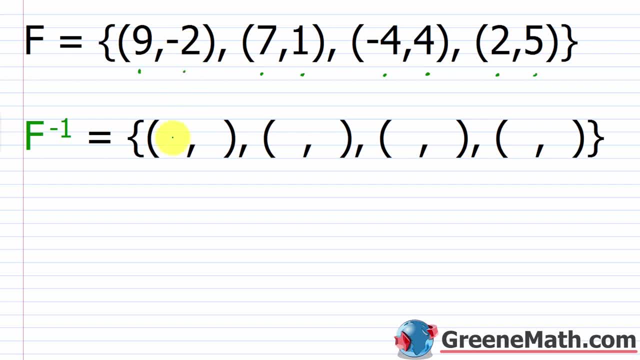 inverse. Again, you just swap the x and y values. So negative 2 becomes the x value here, So negative 9 becomes the y-value, You know so on and so forth. So this would be 1,, 7,, 4, negative 4,. 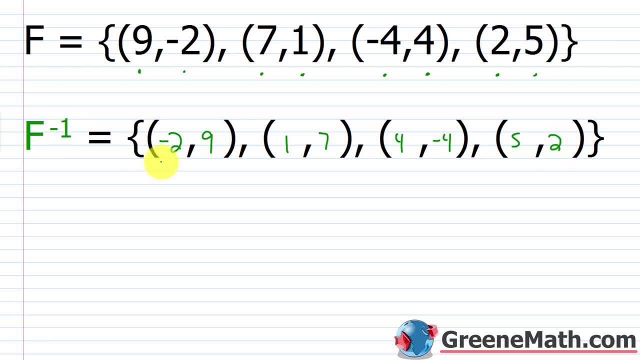 and then 5, 2.. So f inverse contains the order of pairs negative 2,, 9,, 1,, 7, 4,, negative 4, and 5, 2.. So the domain of f, which consists of 9,, 7, negative 4, and 2, became the range of f. 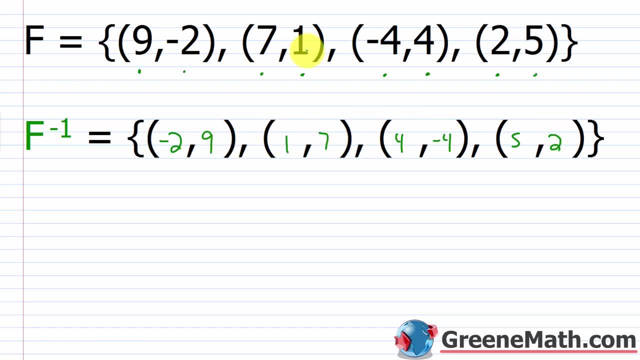 inverse right- 9,, 7, negative 4, and 2.. The range of f, which consists of negative 2,, 1,, 4, and 5, became the domain of f: inverse right- Negative 2,, 1,, 4, and 5.. All right, let's take a look at g. 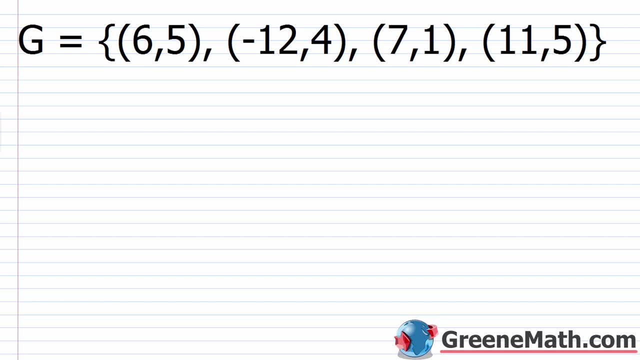 So will g have an inverse. So the first thing is: is g a one-to-one function? I see you have an x value of 6, negative 12,, 7, and 11.. So no duplicate x values there. so we're good. So we think about. 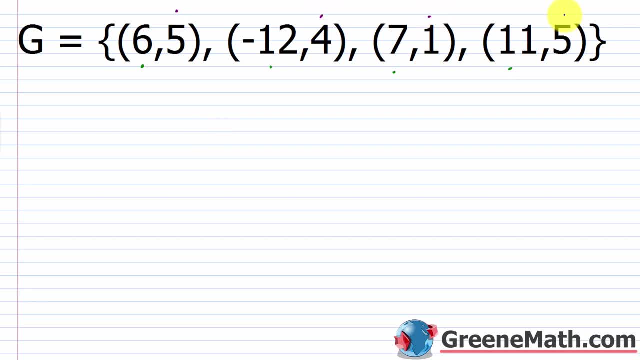 duplicate y values. So you have 5,, 4,, 1, and then 5 again. So here this fails the definition of a one-to-one function. So it's a one-to-one function. So it's a one-to-one function. So it's a one-to-one. 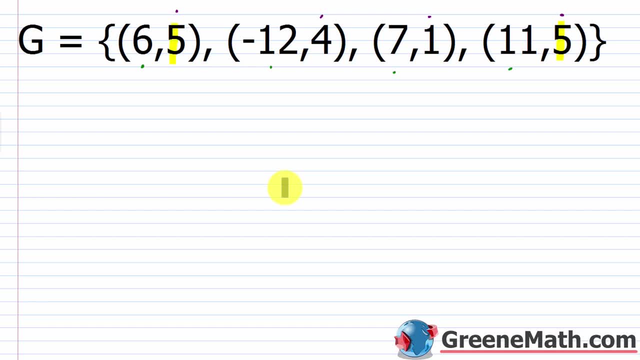 function. It's a function because each x is associated with only one y, but it's not a one-to-one function because each y value- in this particular case 5, is not associated with one unique x value. right, The y value of 5 is associated with or linked up to 11, and then 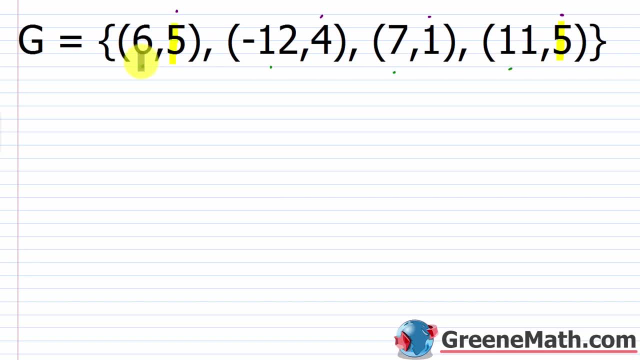 also 6.. So this fails the definition of a one-to-one function And the reason you want something to be one-to-one. think about if I tried to make the inverse of g. So let's say I had g inverse like this and you set it up: Well, I reverse everything. So this is. 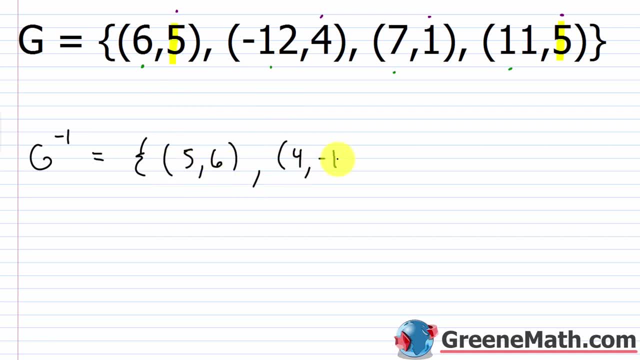 5, 6.. This is 4, negative 12.. This is 1,, 7.. And then this is 5,, 11.. So you say, hey, if x is 5,, what's y? when we think about the inverse? Well, it could be 6,, but it could also be 11.. So in 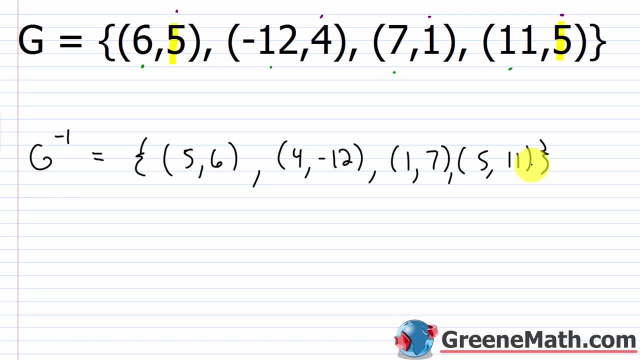 other words, it's got to be a one-to-one correspondence to say, hey, x is 5, here, y is going to be this right. In this case, x is 5.. We don't know whether to say y is 6 or y is 11.. 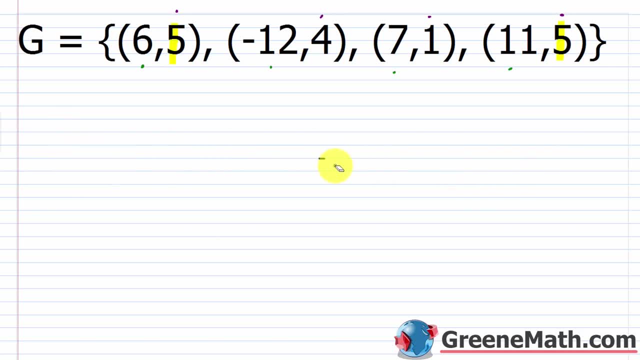 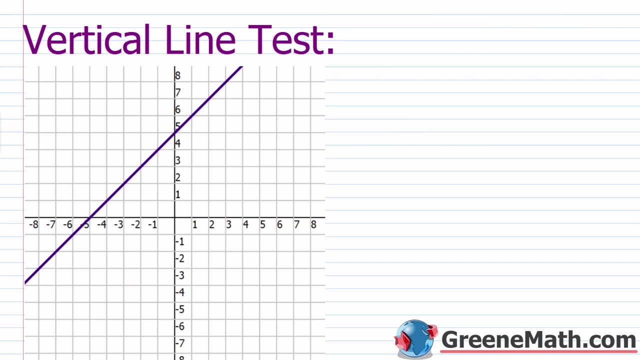 So it's not a one-to-one function and so it will not have an inverse, So we'll just put not a one-to-one function, All right. So let's talk a little bit about how you would go about determining if you have a one-to-one function or not. So you'll recall that. 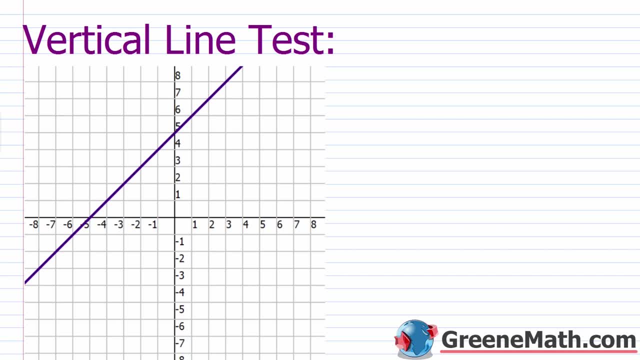 we talked about functions, We had this idea of a vertical line test. Essentially, if a vertical line hits the graph in more than one place, we do not have a function. This would tell us that the same x value corresponds to more than one y value. If we take a look at something like a linear 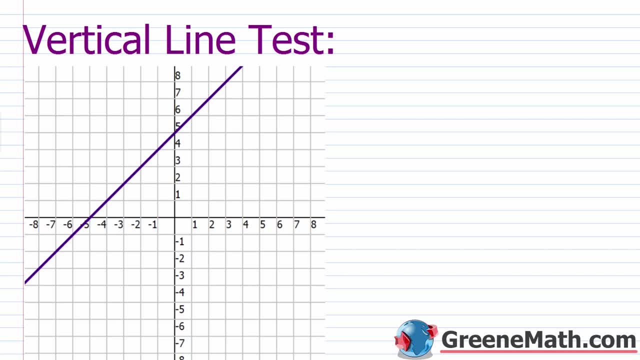 equation. we know this is a function. I could draw as many vertical lines as I want, and I'm never going to impact the graph in more than one spot. So you see here, each vertical line, which is a one-to-one function, is a one-to-one function, So I'm going to draw as many vertical. 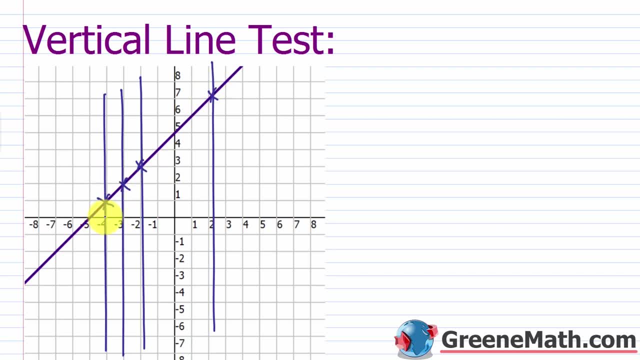 lines as I want, and I'm never going to impact the graph in more than one spot. So you think about your x value. it's associated with one and only one y value there, So this is a function. Here's an example of something that's not a function. Clearly, this would fail the vertical. 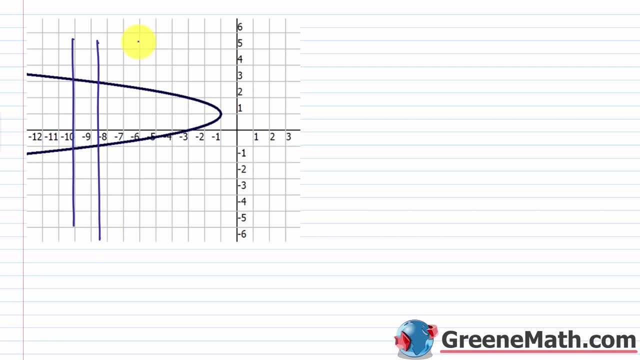 line test. So if we look at all these vertical lines, you could see that for a given x value, we have more than one y value that's associated with it. So for each x, we have more than one y value associated with it. So this is not a function. So this is not a function, All right. so now let's. 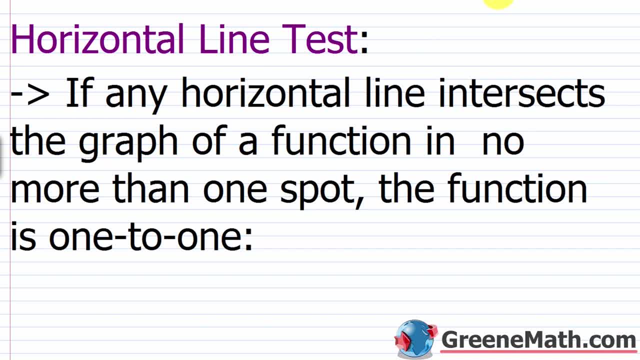 talk about the horizontal line test. So this is similar in concept to the vertical line test, but the horizontal line test is going to tell us if we have a one-to-one function We think about a horizontal line. A horizontal line is a function that is a one-to-one function. So if we think about 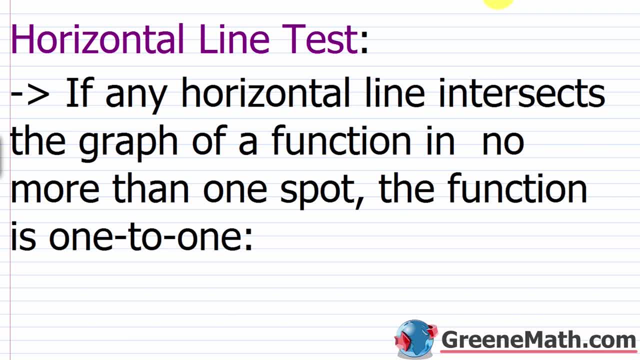 a horizontal line. a horizontal line is y equals something, So it's the same y value. If it impacts the graph in more than one location, that same y value is going to correspond to more than one x value, And so we don't have a one-to-one function. So we can say here: if any horizontal line, 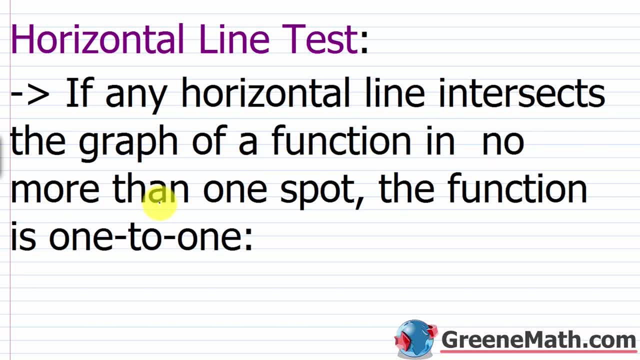 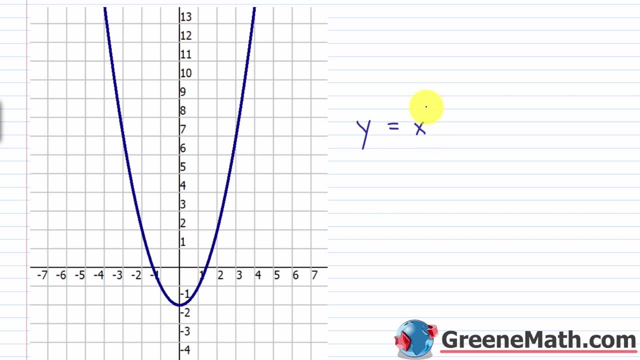 intersects the graph of a function in no more than one spot, the function is one-to-one, right. If it does impact the graph in more than one spot, the function is not one-to-one. So this is the graph of f of x, or you could say: y is equal to x squared minus two. 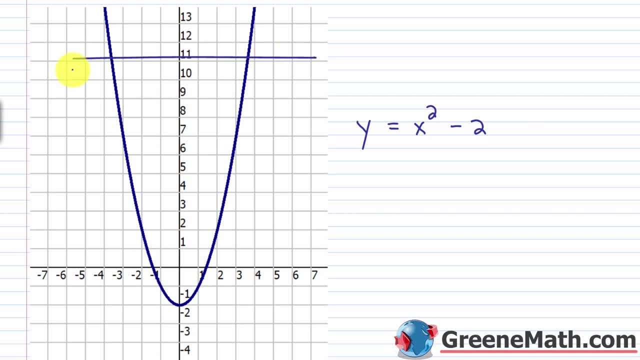 So obviously this is not a one-to-one function. So you can look at these horizontal lines and you can see that they impact the graph more than once in each case, And so this fails the definition of a one-to-one function, because for the y values you're given, they have more than one x value. 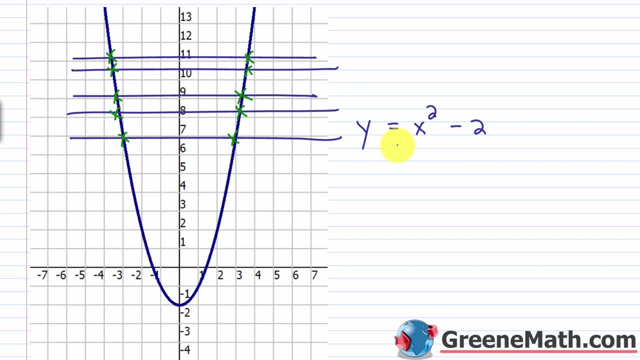 associated with it. Now you could solve this guy for x and see why that's the case. I can add two to both sides of the equation. That would be: y plus two is equal to x squared. I could take the square root of both sides. If I do that, what happens? I get plus or minus the square root of. 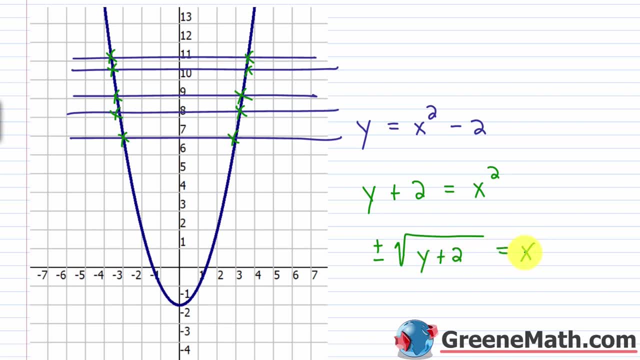 y plus two is equal to x. So think about that. For a given y value, I'm going to now get two associated x values because of this plus or minus operation. Let's pick something easy from the graph. So we know that an x value of three would correspond to: 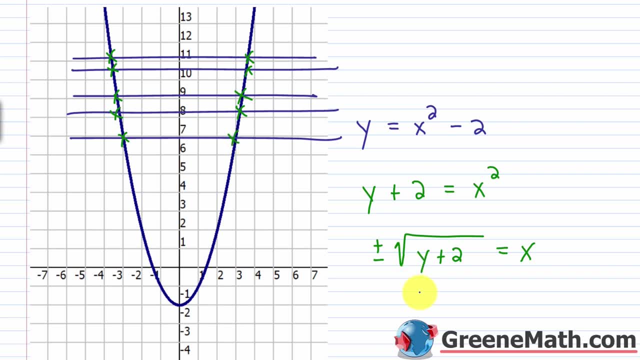 a y value of seven. So if I plugged in a seven for y, seven plus two would be nine. I would have plus or minus the square root of nine. Square root of nine is three, So I'd have positive three or negative three for x, So that y value of seven is associated with an x value of three. 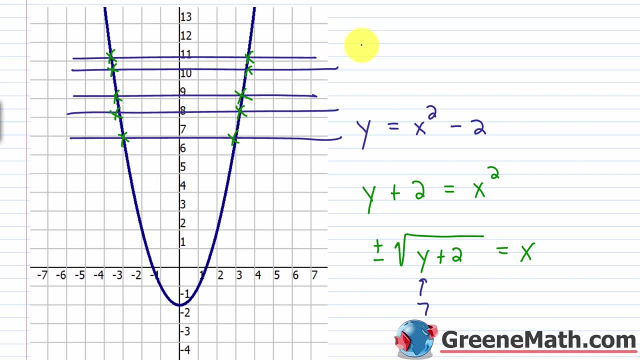 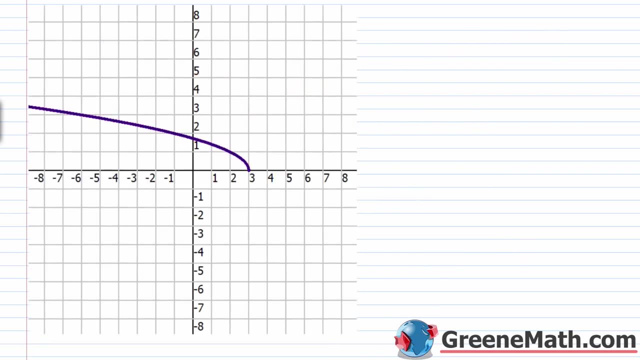 and then also an x value of negative three. So this is not one-to-one. All right, what about this function? right here? Obviously this is a one-to-one function. You can see that each line I drew would only impact the graph in one and only one spot. So 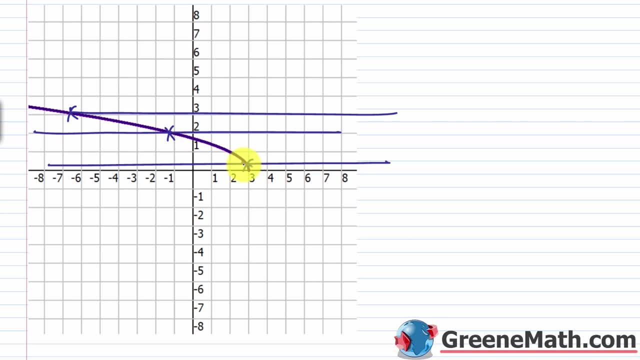 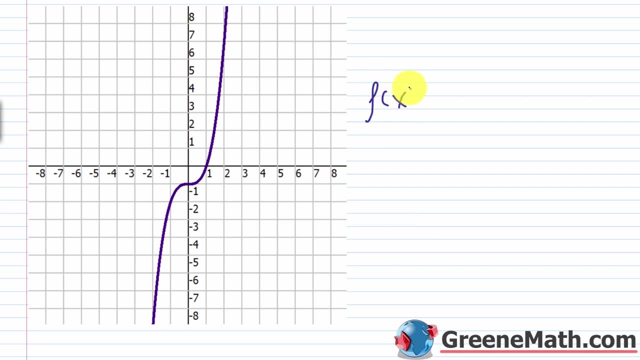 for every y value here there's only one associated x value. All right, so the next graph is one that causes a little bit of confusion. This is the graph of f, of x is equal to x squared minus one. So I'm going to tell you right off the bat: this is a one-to-one function, So I could 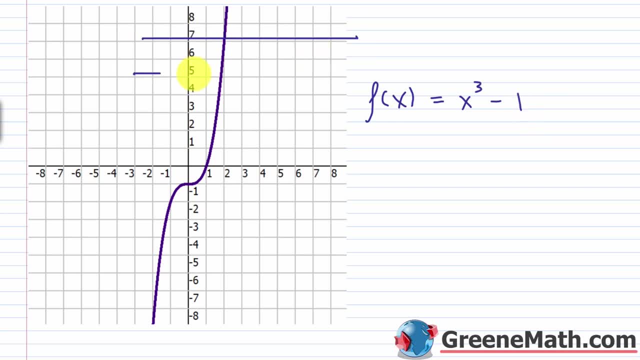 go through and draw horizontal lines And you can see that all these lines would just impact the graph once Where students get confused or where students get tricked here most computer software, most graphing calculators, will draw this part right here, looking semi-flat right. So it kind. 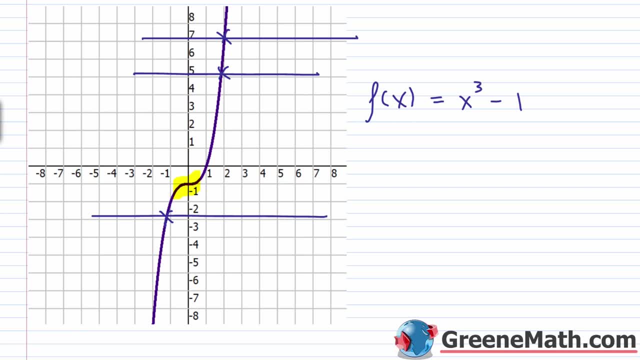 of looks like a horizontal line would impact the graph once. So I'm going to tell you right off the bat: this is a one-to-one function. You can see that each line is only going to impact the graph there in more than one location, But that's not the case If you really just think about this, for 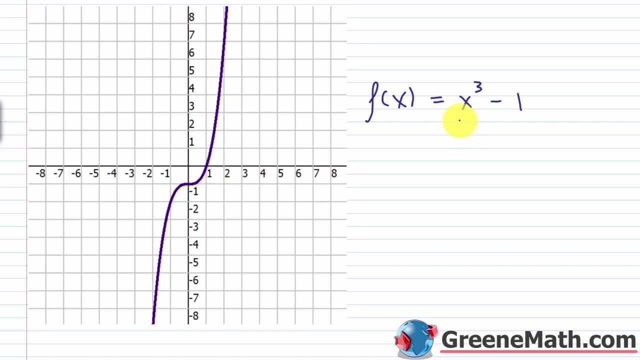 a second when x is zero. okay, when x is zero, y or f of x is negative one. So you have the order pair: zero, comma, negative one. That exists right there. Every value to the left of zero for x, as we move towards negative one, is going to decrease the y value. So this guy is going to 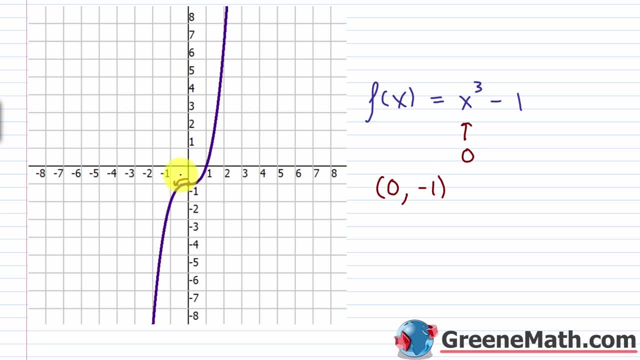 drop this way. It doesn't drop that quickly when you look on the left side of the graph. So if I took something like negative one half and plugged it in for x, I would get a smaller value than negative one, right? This guy's decreasing If I looked at the values between zero and one. 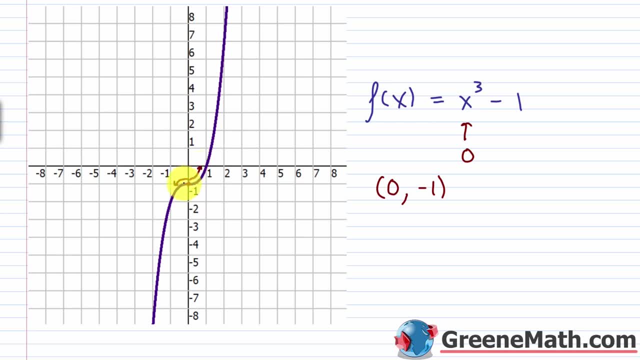 it's the same thing. This guy is increasing here. It looks like a horizontal line right there would impact the graph more than once, but it actually wouldn't. So that's where you got to kind of look at the equation and think about: well, all right if I plugged in something infinitesimally larger. 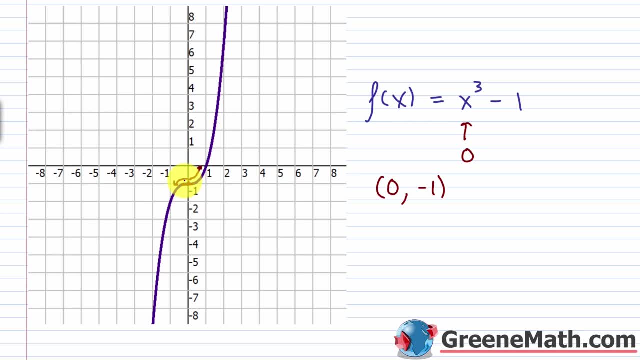 than zero. would I still get negative one If I plugged in something infinitesimally larger than negative one as a result? The answer to that is no. So obviously it's not a horizontal line that would touch the graph in more than one location. So this is a one-to-one function. So this is a 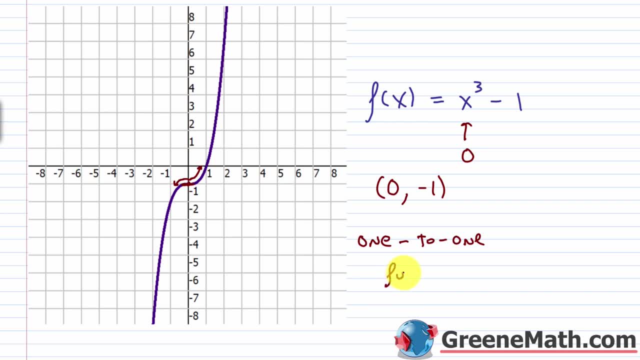 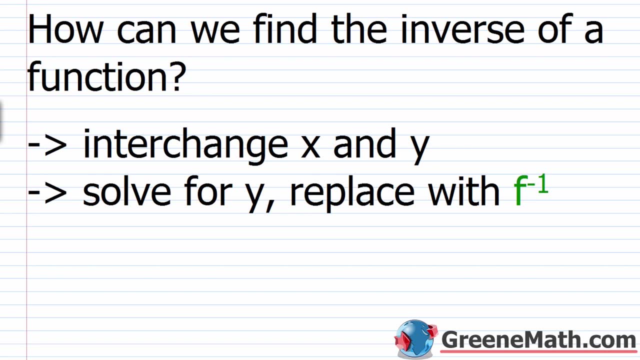 one-to-one function. All right, so now let's get to kind of the main thing, the thing that you're going to see most often in this section. You're going to be asked: how can you find the inverse of a function? I showed you earlier when we talked about that. 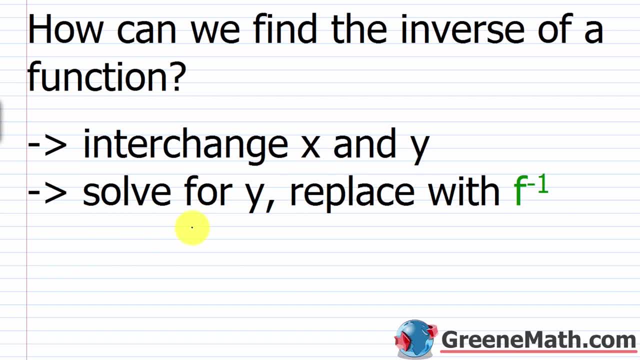 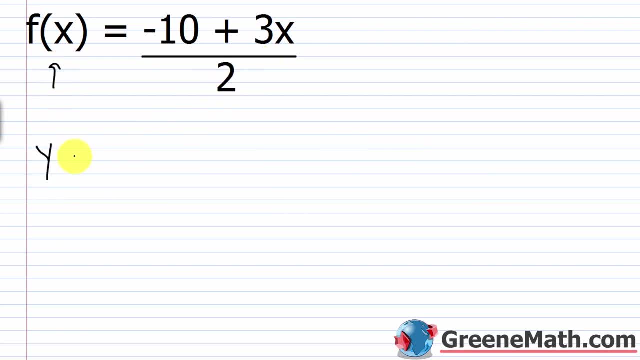 notation. We want to interchange the inverse of a function with the inverse of a function. So I'm going to interchange x and y, solve for y and then replace with f inverse. So I'm going to start out by just replacing f of x with y And then I'm going to say: y equals negative 10 plus. 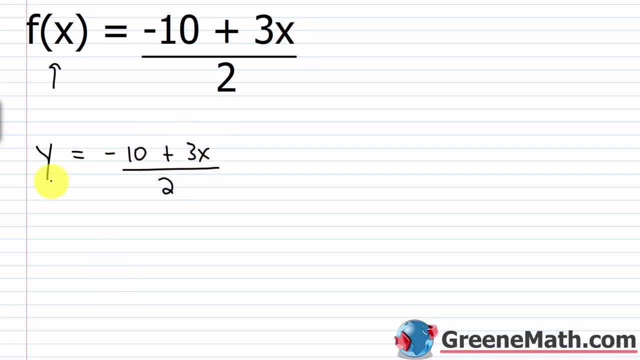 3x over 2.. Now I'm going to interchange y and x. So this would be: x equals negative 10 plus 3y over 2.. So I just interchanged x and y. I didn't do anything fancy Then I'm just going to solve. 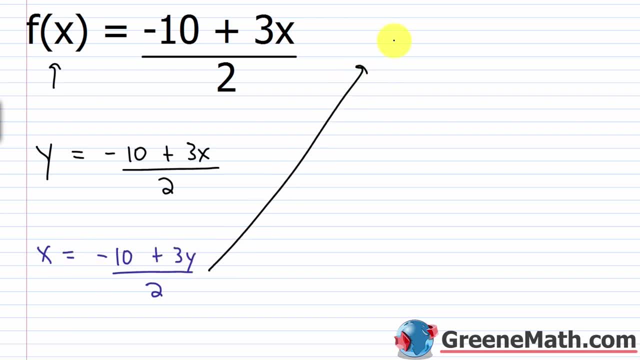 for y. So if I do that up here, I'm going to be able to find the inverse of a function. So I'm going to do that up here. I would multiply both sides of the equation by 2.. So you'd have 2x is. 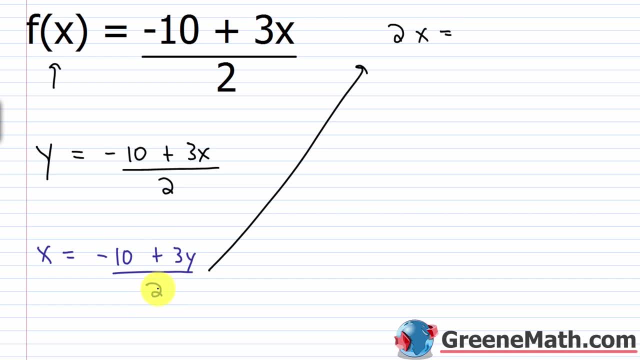 equal to. If I multiply over here by 2,, I would cancel that denominator of 2.. So I would just have negative 10 plus 3y. Then I'm solving for y. So let me add 10 to both sides of the equation. 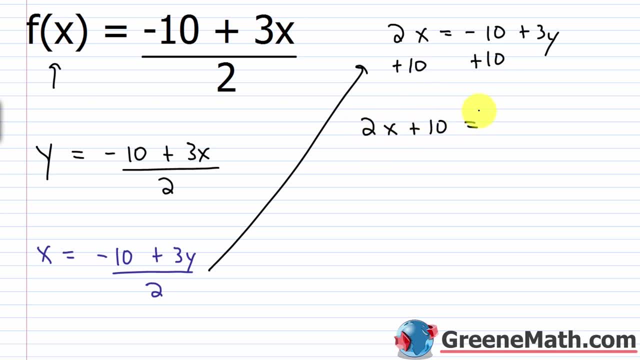 So this is 2x plus 10, is equal to, That's canceled, So just 3y. The last step is to divide both sides of the equation by 3. And I would get that 2x plus 10.. So I'm going to do that over here. 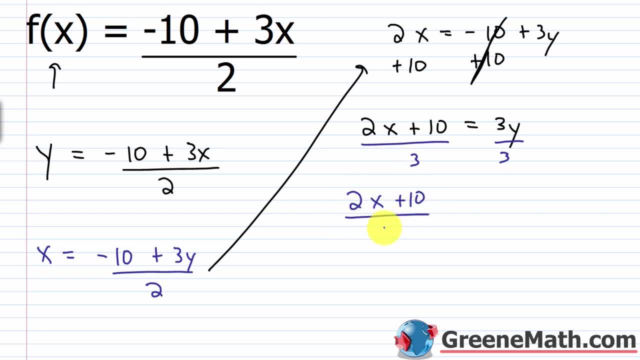 So this is 2x plus 10 over 3 is equal to y. Okay, So let's erase everything real quick. And this guy y, I'm going to now replace with f, inverse, Just to notate that, hey, this guy is the inverse of. 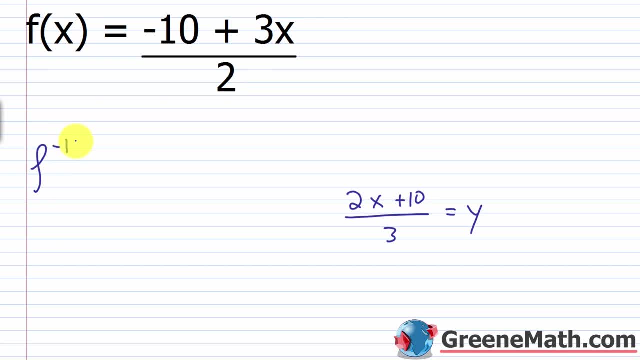 this guy. That's all it is. So f inverse of x is equal to 2x plus 10 over 3.. So these two are inverses of each other. And again, I'm going to do that over here. So I'm going to do that over here. 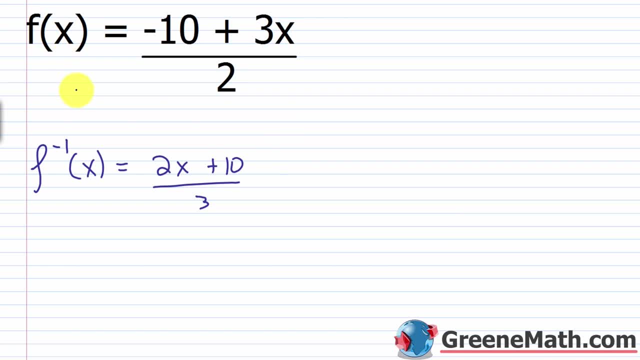 Again. if you wanted to think about how you could prove that to yourself. well, if I plugged in a 4 for x here, So if I had an x value of 4, you'd have 3 times 4, which is 12.. 12 minus 10 would. 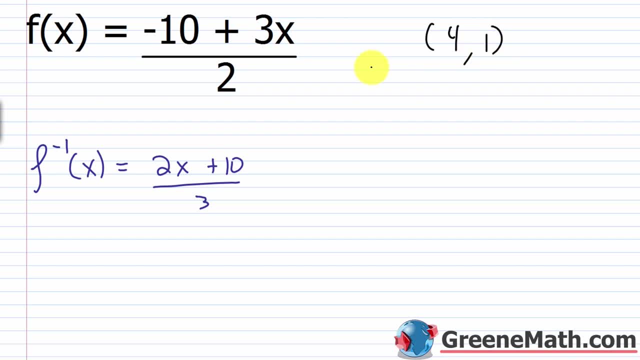 give me 2.. So I'd have 2 over 2, which is 1.. So on this function, we have an x value of 4, a y value of 1.. Remember, the x and y's are interchanged. So if I take a y value of 1 and plug it in for x, 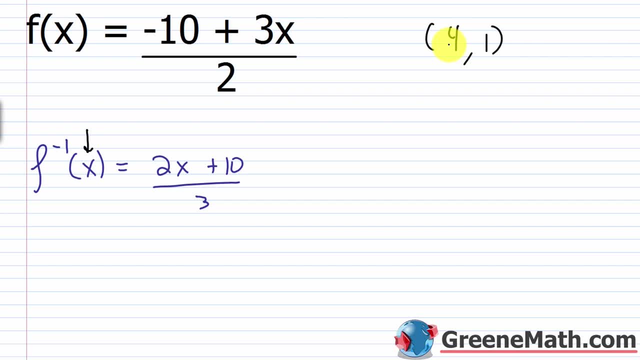 inverse, I should get a result of 4.. So if I plugged in a 1 there, what would I get? 2 times 1 is 2.. 2 plus 10 is 12.. 12 divided by 3 is 4.. So here the ordered pair would be what It would be. 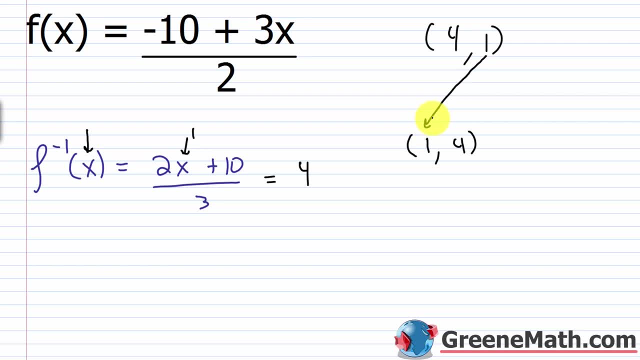 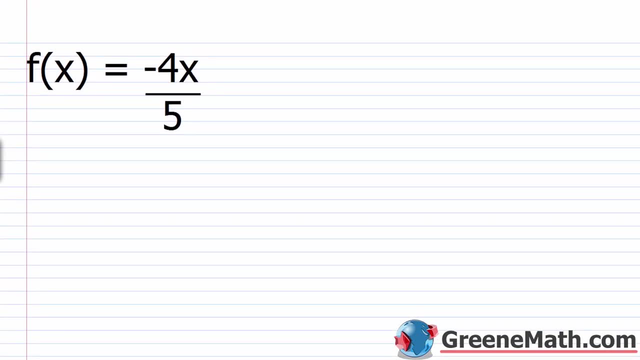 1 comma 4.. Again, the y value became x, The x value became y. So the values here are interchanged. All right, let's take a look at another example. So we have f of x is equal to negative 4.. 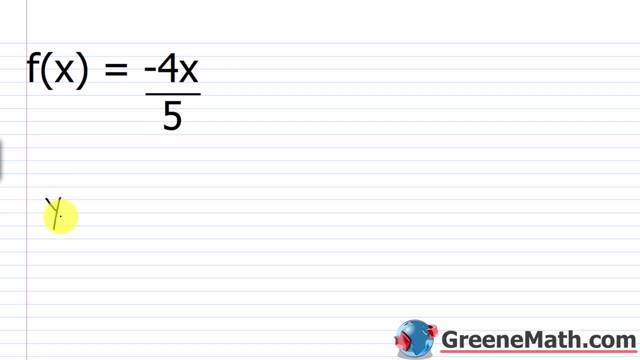 Again, to do this as simply as we can: y equals negative 4 fifths x. We interchange x and y. So we interchange x and y And then we solve for y. So I would just multiply both sides by 5 over. 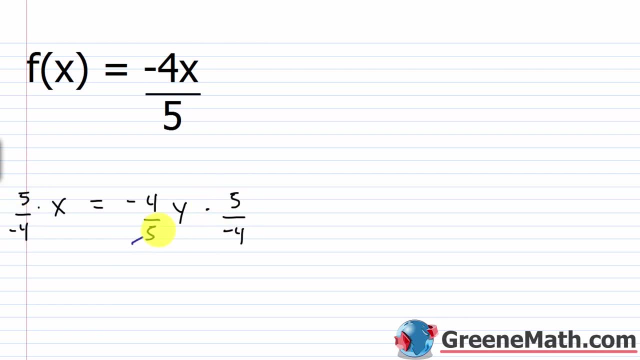 negative 4.. And so this would cancel with this this. with this We'd have: y is equal to negative 5 fourths x. Or we could say: f, inverse of x, is equal to negative 5 fourths x. So if you wanted to check this, let's just choose. 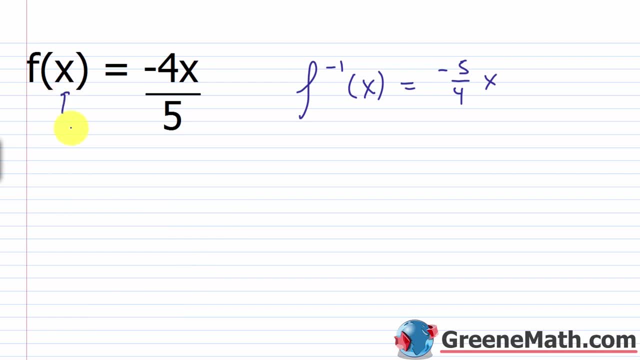 something for x. Let's say we chose, I don't know. let's say 5.. So f of 5 would be equal to negative 4 times 5 over 5. The 5s would cancel. I'd be left with negative 4.. So if I take 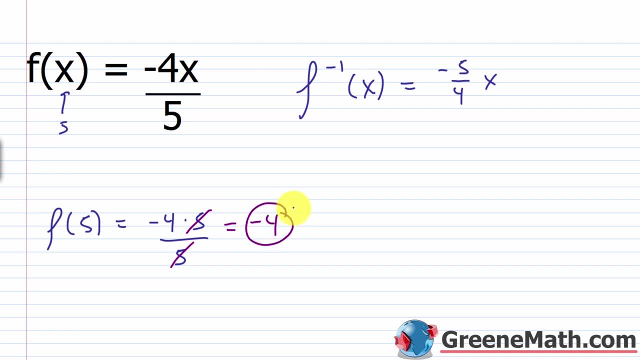 negative 4, which is the y value here, and I plug it in for x here, I should get 5 back. So if I plug in a negative 4 here, this cancels with this And I've got negative 1.. 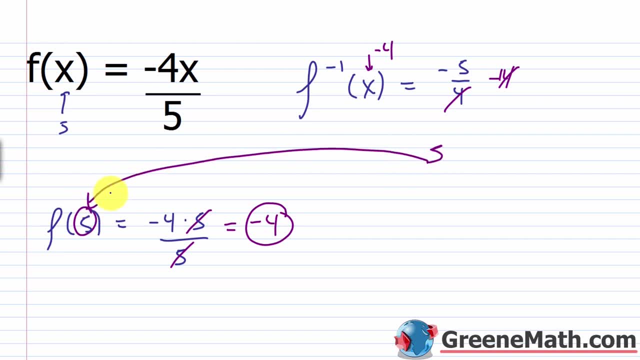 Negative 5 times negative. 1 is 5.. Right, I go right back to that. All right, let's say we saw f of x equals x cubed minus 2.. So again we say: y equals x cubed minus 2.. And I interchange y and x. 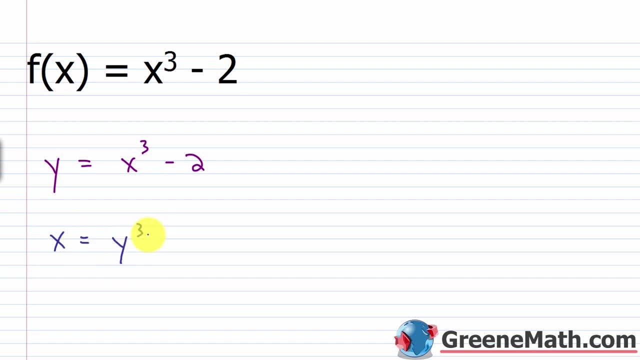 So this would be: x equals y cubed minus 2.. And to solve for y, I would add 2 to both sides of the equation. So that's going to give me x plus 2 is equal to y cubed. And to solve for y, I'm just going to take the cube root of each side. 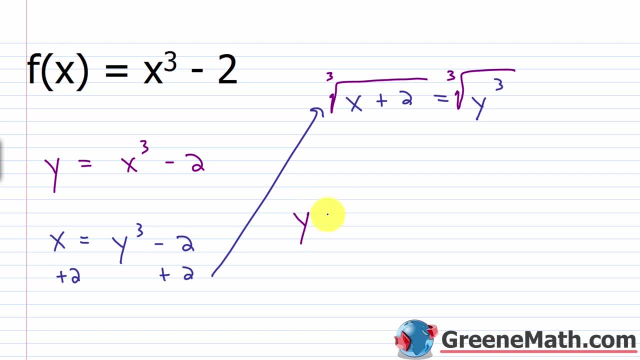 And so what's going to happen is I'll have: y is equal to the cube root of x plus 2.. Let me erase all this. We can do the proper notation. So these two are inverses. So we would say f inverse. 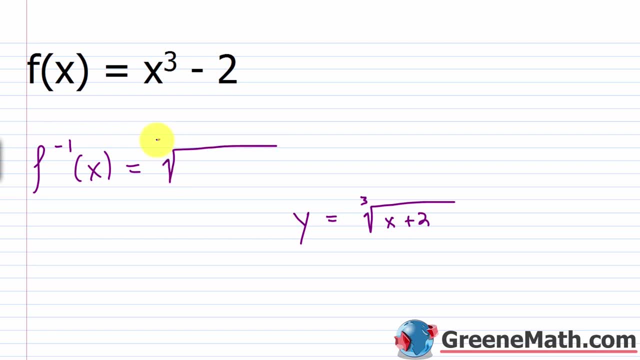 Of x is equal to the cube root of x plus 2.. And again, if you pick a value for x, let's say you pick 3.. So 3 cubed, we know that 3 times 3 is 9.. 9 times 3 is 27.. 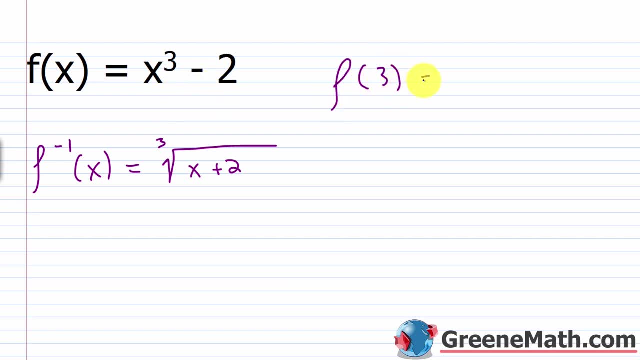 Subtract away 2,, you get 25.. So f of 3 is equal to 25.. So I should be able to take 25 and plug it in for x and get back to 3.. Right, So if I take f inverse of 25,, 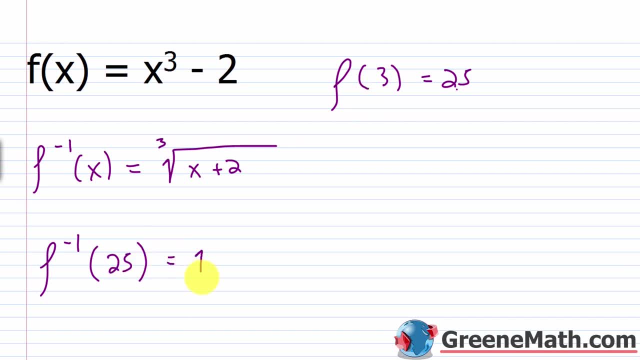 I expect the result to be x cubed minus 2.. So I'm going to subtract away 2.. So I'm going to subtract the result to be 3.. So the cube root of 25 plus 2.. 25 plus 2 is 27.. The cube root of 27 is 3.. 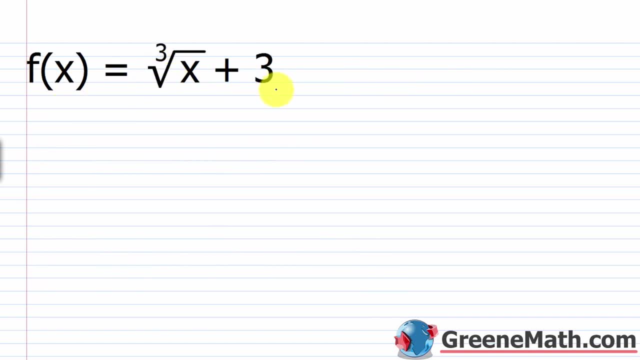 All right, let's say we saw, f of x equals the cube root of x plus 3.. Again we'll say y equals the cube root of x plus 3. Interchange x and y. So x equals the cube root of y plus 3.. So let's. 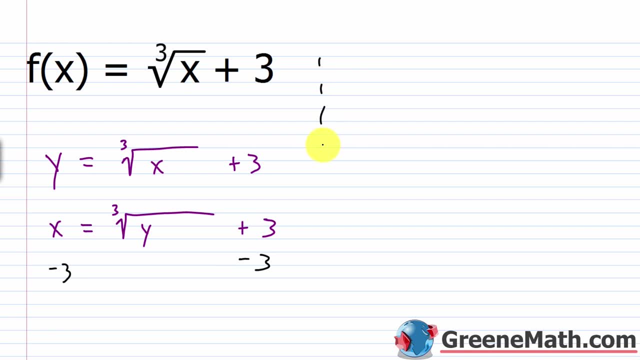 subtract 3 away from each side of the equation, We will have x minus 3 is equal to the cube root of y. And then I would just cube each side of the equation So I would have y is equal to the quantity x minus 3 cubed. So let's erase all. 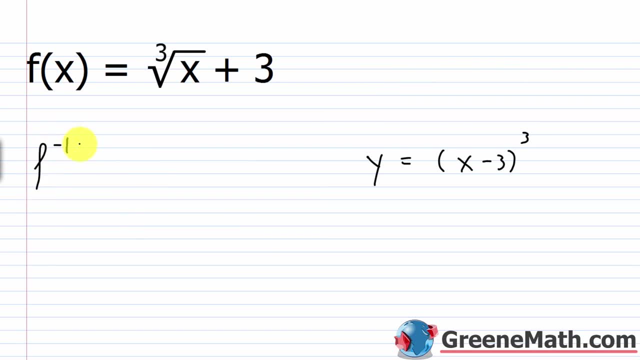 this And we'll use the proper notation. We'll say f inverse of x is equal to the quantity x minus 3.. And this is cubed. Let's take a look at another one. So suppose we see f of x equals 3 over x minus 1 minus 2.. 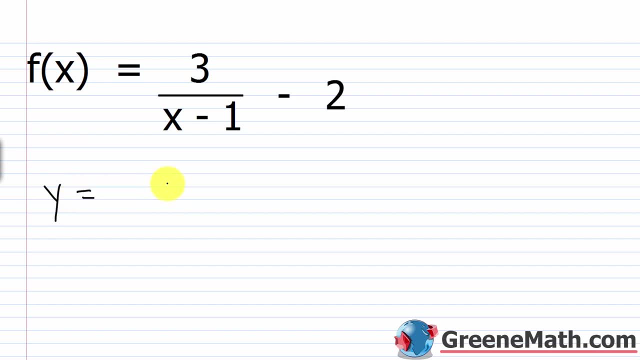 So again, to find the inverse, we'll say y equals 3 over x minus 1 minus 2.. Swap out x and y, So let's just say this is y and this is x. So how do we solve for y now? Well, we've got to add 2 to. 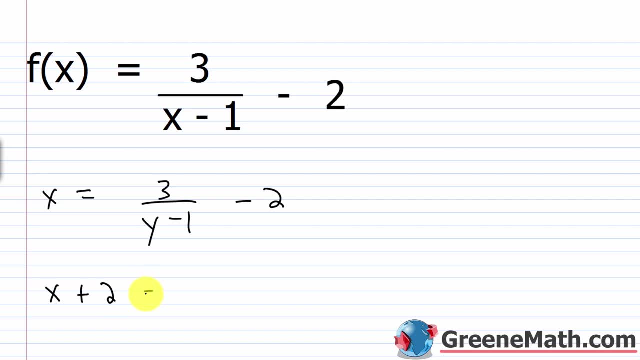 the equation- So we'd have x plus 2- is equal to 3 over y minus 1.. So now let's multiply both sides of the equation by the quantity x plus 3 over x minus 1.. So let's take a look at another one. 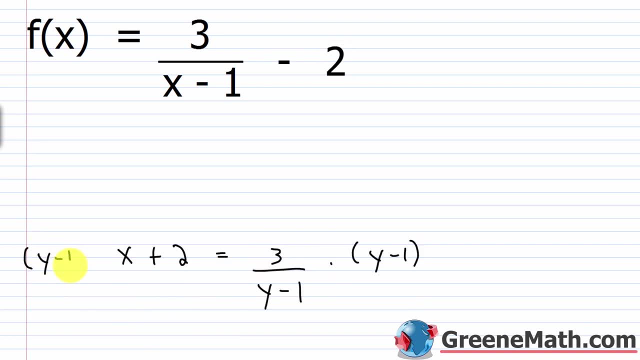 So what would that give me? Well, this would cancel over here. I would have the quantity y minus 1 times the quantity x plus 2 is equal to 3.. So let's do 4 here. y times x is xy The outer. 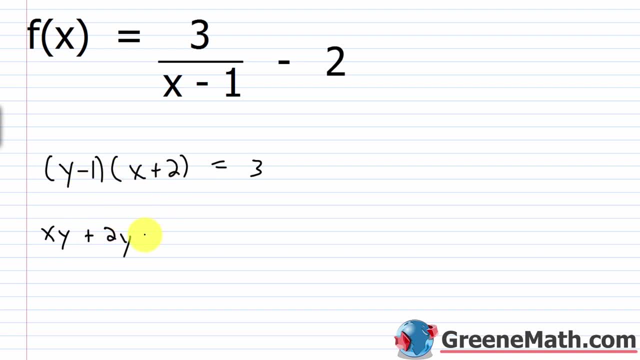 y times 2 is plus 2y. The inner negative 1 times x is minus x And the last negative 1 times 2 is minus 2.. This equals 3.. So everything with a y on the left, everything without a y on the right. So let's add x, Let's. 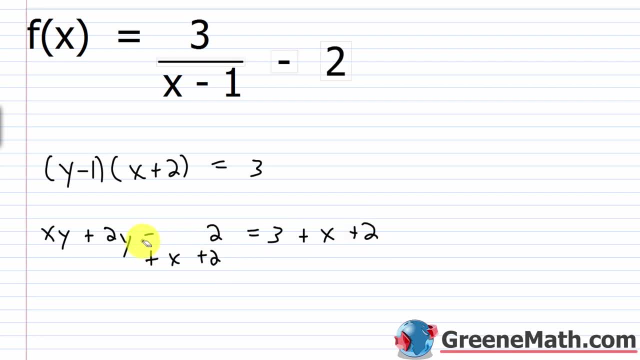 add 2 to both sides of the equation, So that would go away. And then let's factor out a y, So I would have y times the quantity x plus 2 there. So we would have y times the quantity x plus 2.. And so what we would do here is just divide both sides of the equation by x plus 2.. 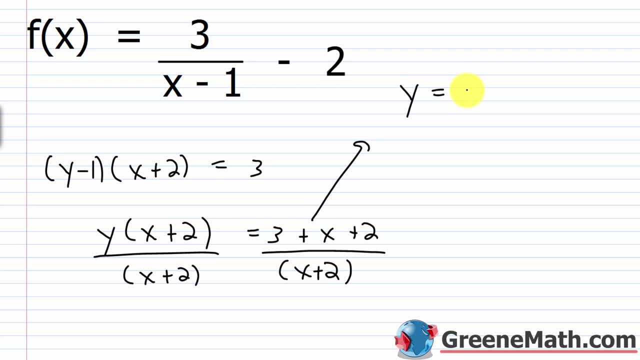 That's going to give us what y is equal to you would have. we'll reorder this to x plus 5, right, because we have x plus 3 plus 2.. 3 plus 2 is 5 over x plus 2.. And again, to notate this: 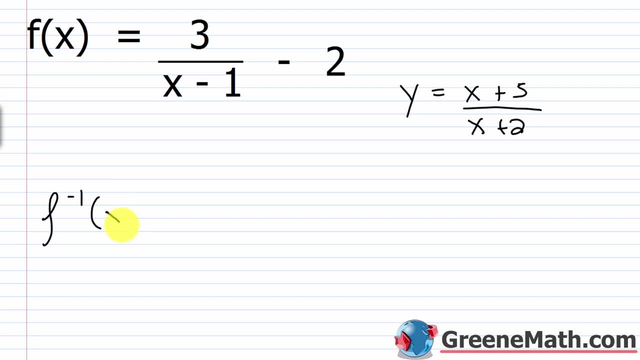 properly. we'll say f inverse of x is equal to x plus 5 over x plus 2.. And again you can choose a value for x. plug it in the original function, you'll get a y. Take that y value. plug it in for x in the inverse and you'll get your original x value. 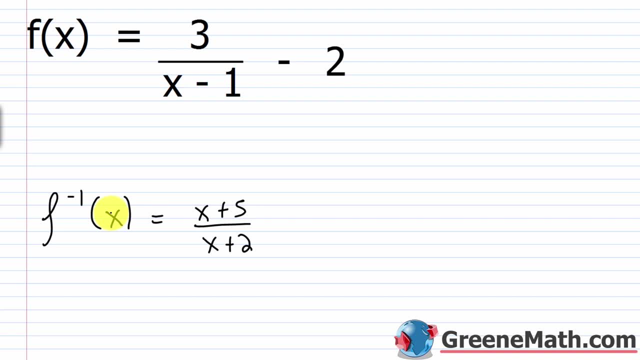 back. So as an easy example, let's say x was 4.. So f of 4 would be what? Plug in a 4 there. 4 minus 1 is 3,, 3 over 3 is 1.. So you'd have 1 minus 2, which is negative 1.. So if I plug in 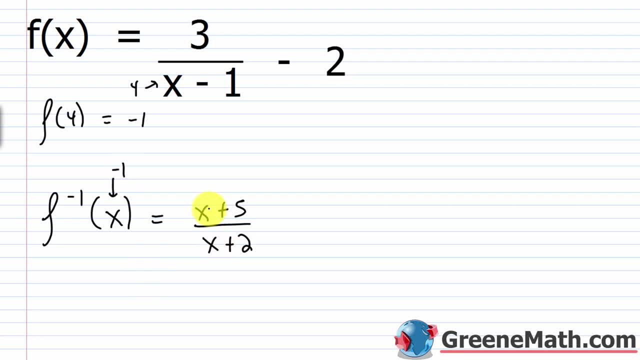 a negative 1 or x. in this inverse, negative 1 plus 5 is 4, right, So this would be 4 over negative 1 plus 2 is 1.. 4 over 1 is 4, so I'm right back to 4.. Hello and welcome to Algebra 2, Lesson 69.. 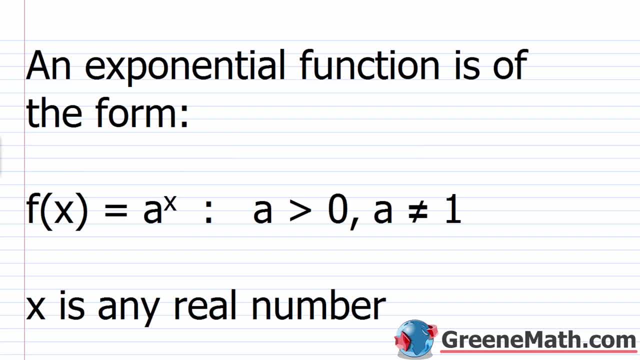 In this lesson we're going to learn about exponential functions. So an exponential function is of the form we see here that we have. f of x is equal to a, which is our base, raised to the power of x. So what makes this a little bit different for us is that we've never 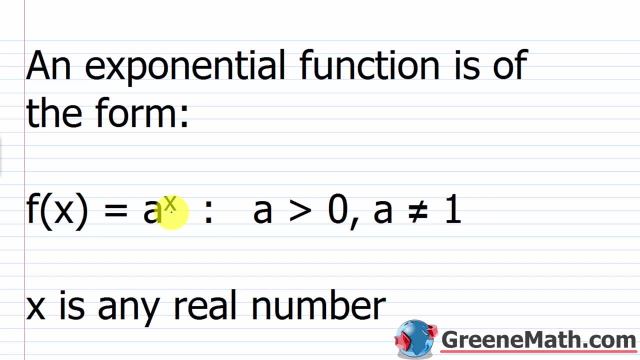 seen a variable involved in the exponent before. So what we'll do here is we'll define a to be any number that is larger than 0, and it's not allowed to be equal to 1.. The reason we put these restrictions on the base is so that we can say that x is any real number And you can just: 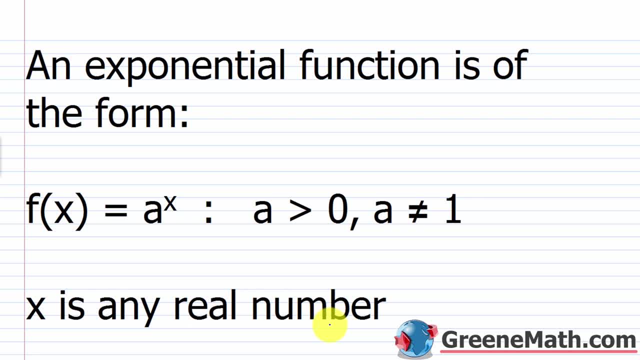 think about for a moment why you need those restrictions on a to make this all work out. Let's say a was allowed to be some negative value. Just to make it simple, let's say it's negative t. So if I had negative 2 as my base and I raised it to I don't know, let's say the number 3,. 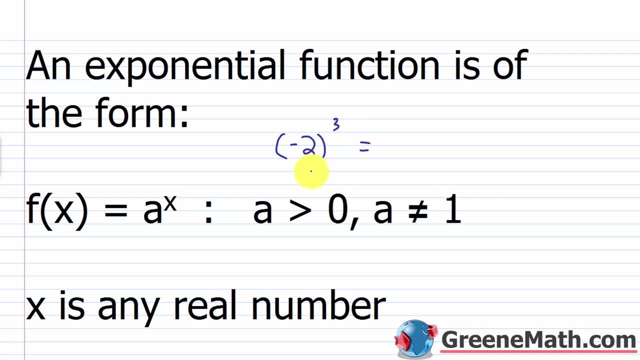 you'd say, okay, there's no problems there. Negative 2 cubed or negative 2 to the third power is negative 2 times negative, 2 times negative 2, which we know would be negative 8.. So that's all. 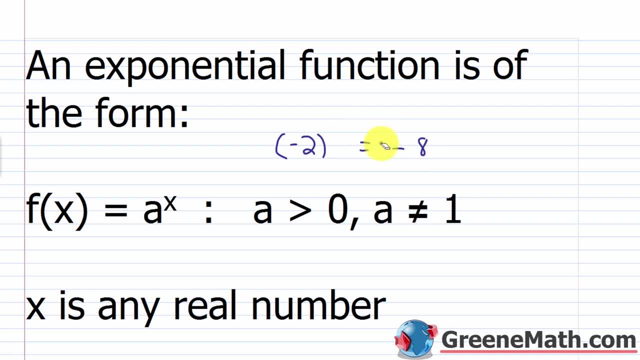 fine. But what if we said: I want negative 2 raised to the power of one half or one fourth or something like that? Well then, this is equal to the square root of negative 2. And although we can deal with this using the complex number system, the answer is not real right. So if 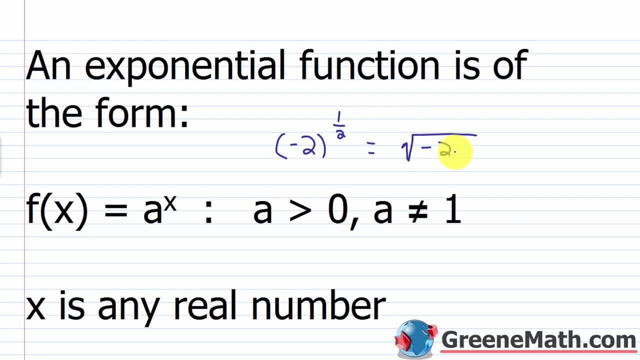 we're dealing with just real numbers. only we want to restrict a to again be greater than 0, and it's not allowed to be equal to 1.. Now let's talk about why it can't be 0. If you think about having 0 as your base, if I raise 0 to some positive value, 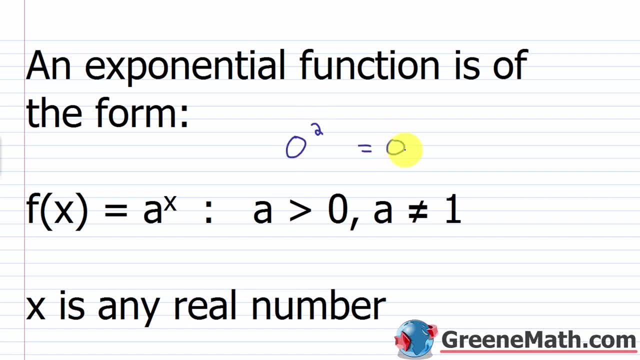 let's say I square it, 0 squared, we know it's just 0. So that's all fine, But I can't raise 0 to the power of 0. That's undefined. And I can't raise 0 to a negative value. 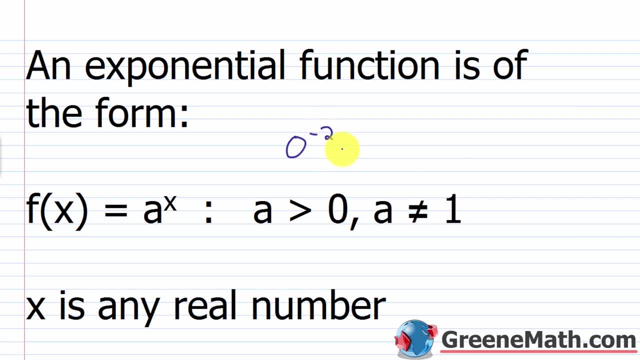 because if I did something like 0 to the power of negative 2, we know this is 1 over 0 squared, and this is 1 over 0, which is undefined, Undefined. So that's why we have these restrictions. 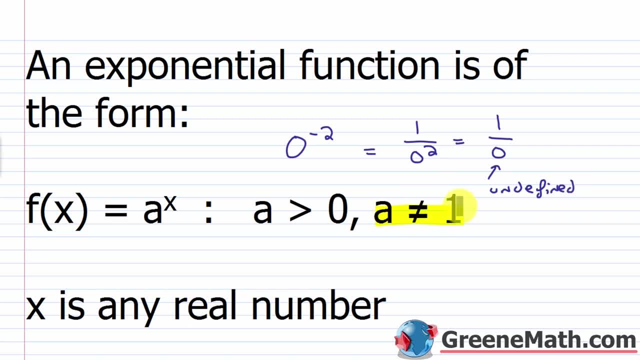 Now let's cover this last one here, where we say a does not equal 1.. Why do you think a, the base, is not allowed to be equal to 1?? Well, we would no longer have an exponential function, We would have a linear function, You might say. well, why is that the case? 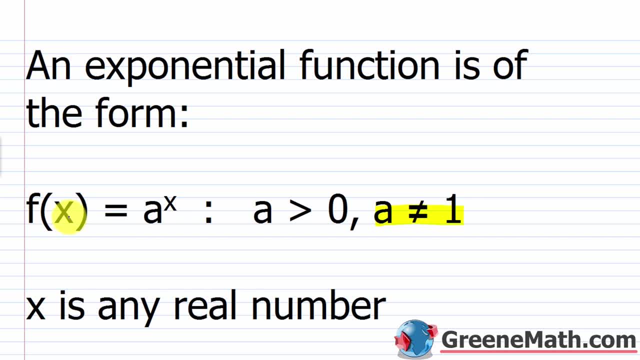 Well, if I say f of x, to make this really simple, instead of f of x, let's just say this is: y is equal to a. I'm just going to replace that with 1, raised to the power of x. So just think. 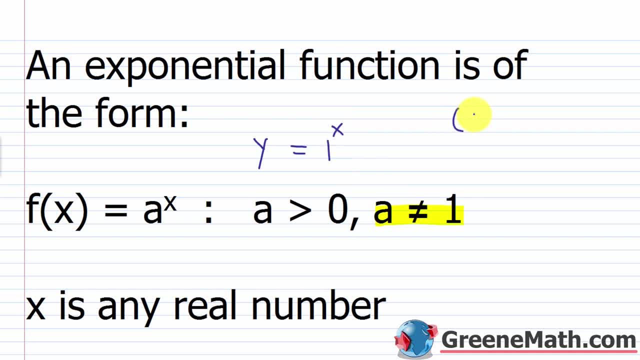 about some ordered pairs? Let's just do 2.. Let's say I picked 2 for x. What would y be? 1 squared is 1.. So y would be 1.. Let's say I picked- I don't know- 10 for x. 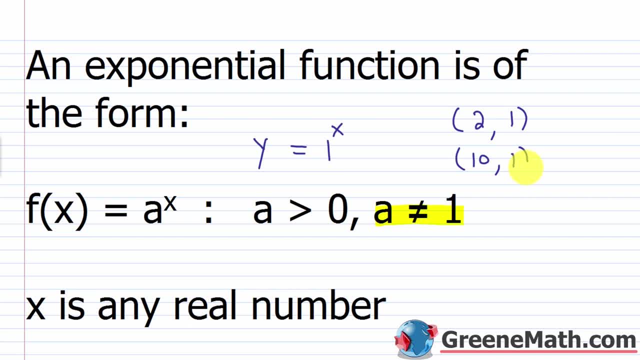 1 to the 10th. power is 1, right, So y would be 1.. You can choose any value you want for x. It doesn't matter Anything in the real number system. When you take 1 and you raise it to a real number, you're going to get 1 back. So 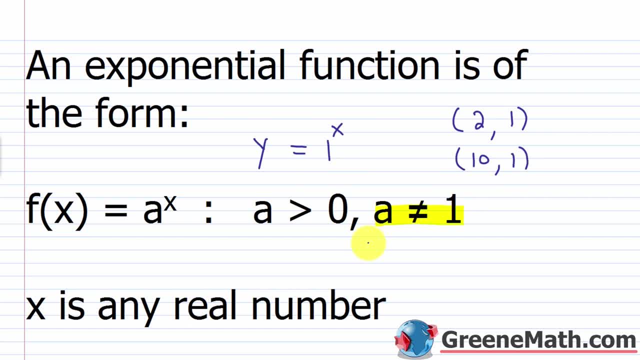 what ends up happening is you could basically say: this is a horizontal line. right, It's the horizontal line. y equals 1.. Or to make it match this format here, we could just say: f of x is equal to 1, right, This is a horizontal line that would impact the y-axis at the point 0,. 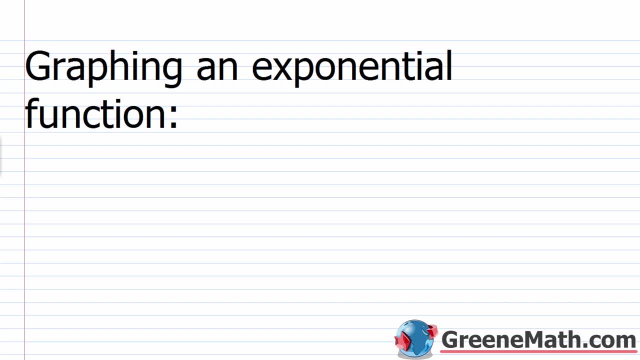 1. So there's kind of two things we're going to talk about in this lesson. The first thing is how to graph an exponential function. We'll spend a little bit of time on that And then we'll move into solving exponential equations. So for graphing an exponential function, just a little bit of. 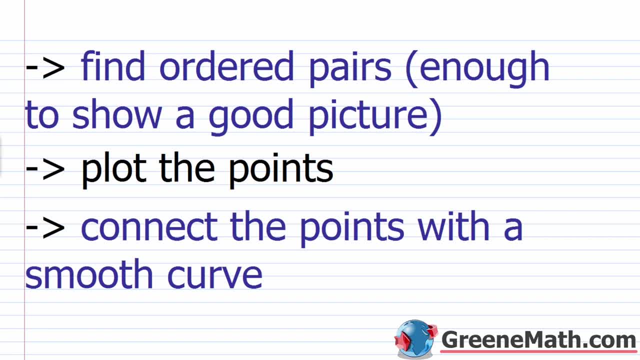 background here. The first thing you would do, just like if you were graphing anything else, you would find some ordered pairs again enough to show a good picture. You'd plot the points like you always do, And then you connect the points with a smooth 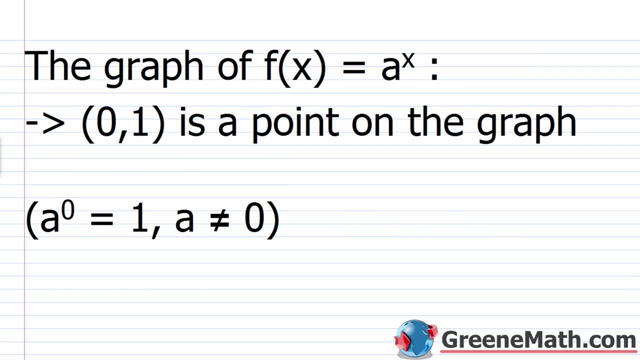 curve. Again, I say this in a lot of videos: when you freehand draw things, if you're going to do a smooth curve, you're going to do a smooth curve. If it's not a line, it's usually going to be pretty inaccurate, right. So you want to stick to. 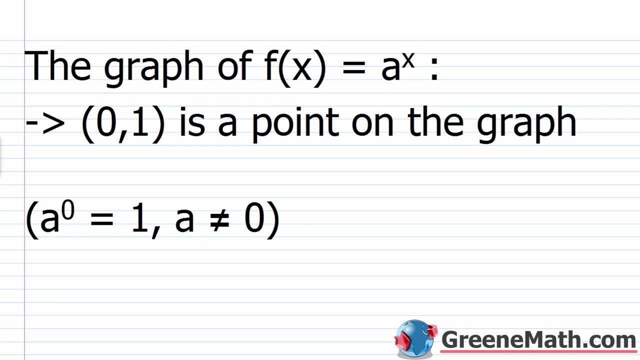 just using this for a conceptual tool. If you actually need to graph something to look at it, you'd probably want to use either computer software or your graphing calculator. So let's start out with the graph of. you have f of x equals a to the power of x. So this kind 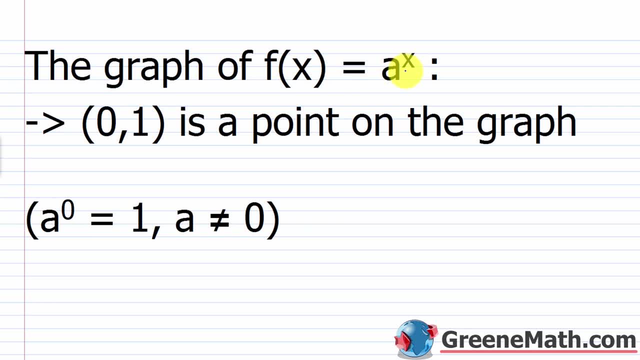 of generic form that we get presented in our textbook. So the first thing is that 0, 1 is a point on the graph. Again, this is the x value, This is the y value. So, in other words, if I plugged in a 0 for x, a to the power of 0 is going. 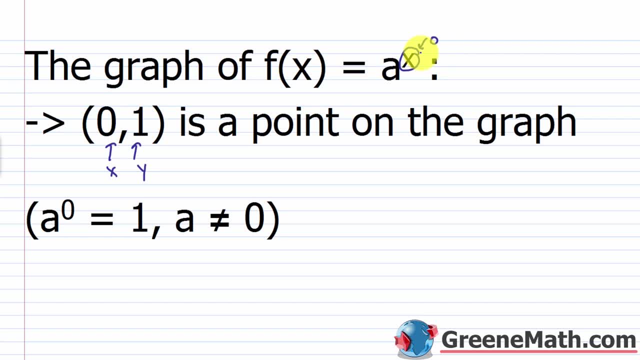 to give me 1, because any non-zero number raised to the power of 0 is going to give me 1.. And remember, we restricted a to be greater than 0. And we also restricted a to not be equal to 1.. 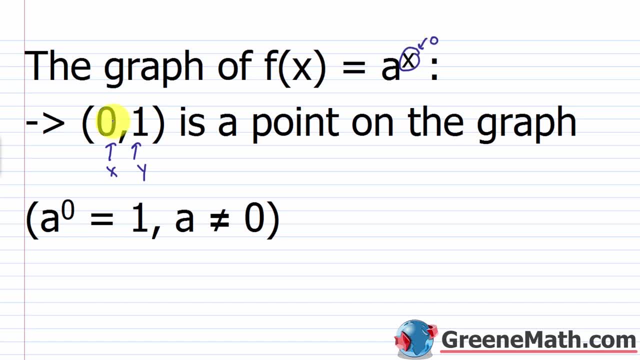 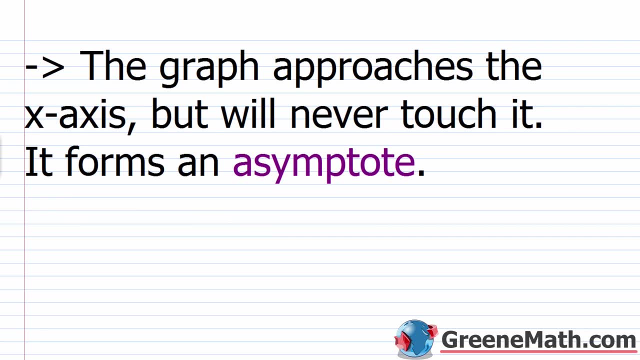 So, following those restrictions, we know if we plug in a 0 for x, we would get a 1 as a result for y. All right, so this is a very important feature when you deal with exponential functions. The graph approaches the x-axis, So it comes very, very close, but it will never touch. 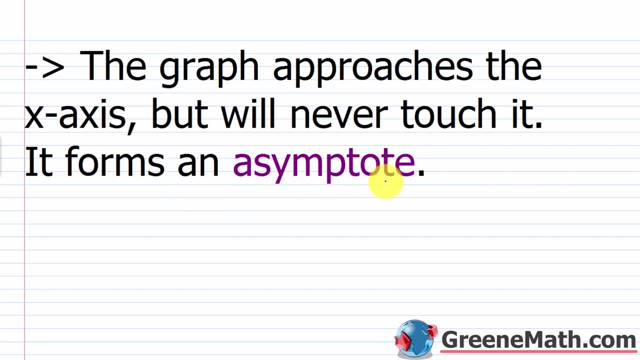 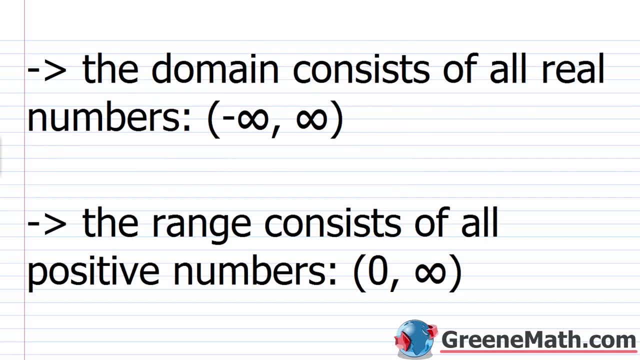 it, It forms something known as an asymptote, And we talked about those before, when we were dealing with rational expressions. So now the domain, which is the set of allowable x values, consists of all real numbers. So, again, because we restricted a, we could say that we can choose. 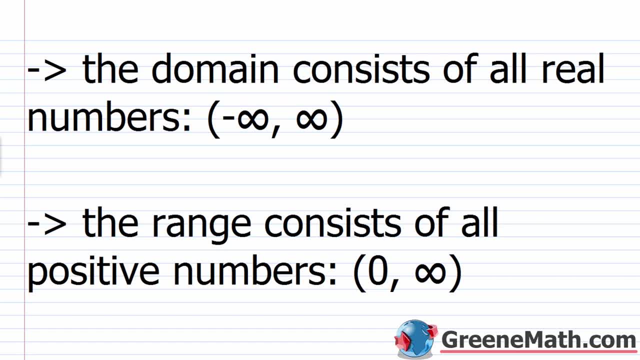 any value in the real number system, from negative infinity to positive infinity, as our input for x, Then the range or the output- the values that we can use for y or for f- of x consists of all positive numbers. So 0 is not involved in that And you can see the way that. 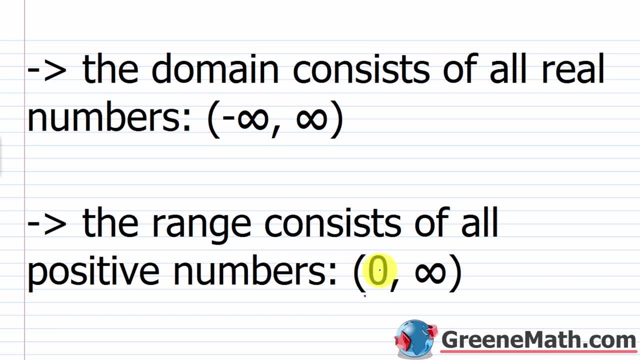 this interval notation is set up Again. if you're using a parenthesis next to 0, it says 0 is not included, but anything larger is. So anything larger than 0 could be 0.000000001.. Okay, if it's larger than 0, it's acceptable. Out to positive. 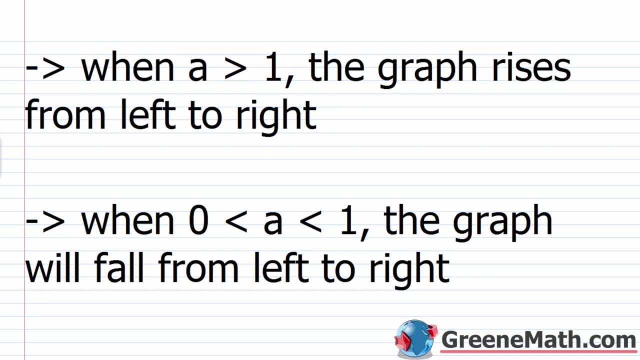 infinity. All right. so when a, your base is greater than 1, the graph rises from left to right. So you're going to see it kind of over to the left As you come from that direction and going to the right, you're going to see it just hockey stick itself up And you'll see an example. 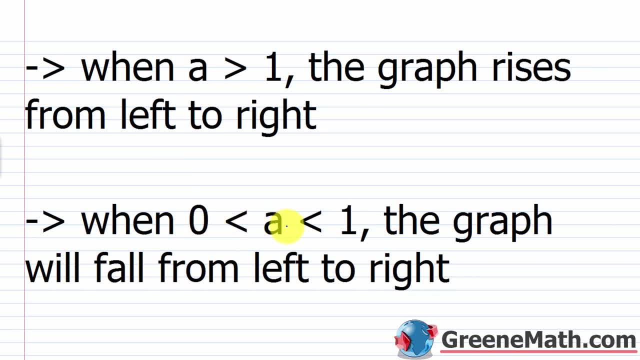 of this in a second. Then, when a is greater than 0 and less than 1,, the graph will fall from left to right. So, in other words, it will start out at a higher point and it will decrease as it moves to the right. All right, so let's take a look at a few. 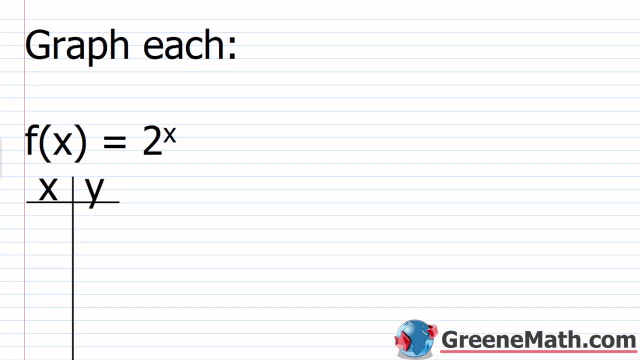 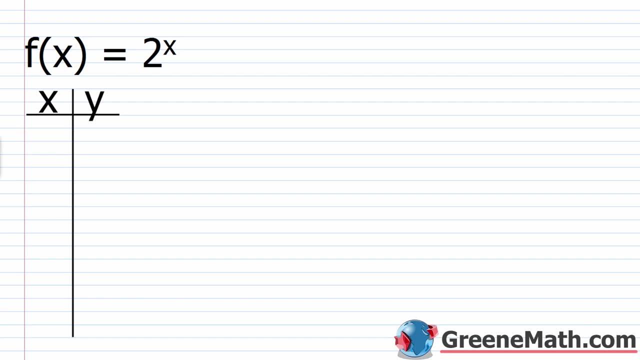 graphs now. So we want to graph each And again. if we're doing this by hand, it's going to be just an approximation, right? We're just doing this to get a little practice on what it would look like. It's not going to be 100% accurate. So f of x is equal to 2 to the power of x. 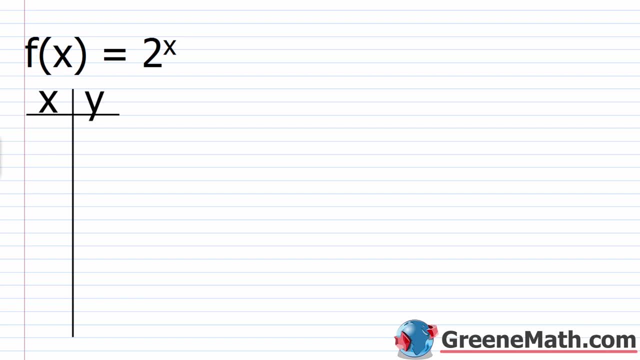 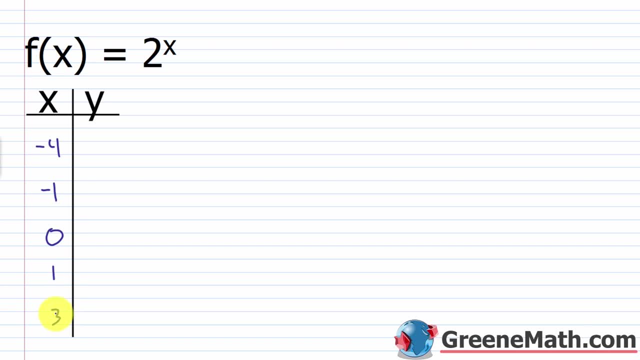 with 1. And I'm going to go with 3.. All right, so 0 comma 1. we know is a point on all of these. We talked about that a minute ago, So I can go ahead and just fill this out and say it's 0 comma. 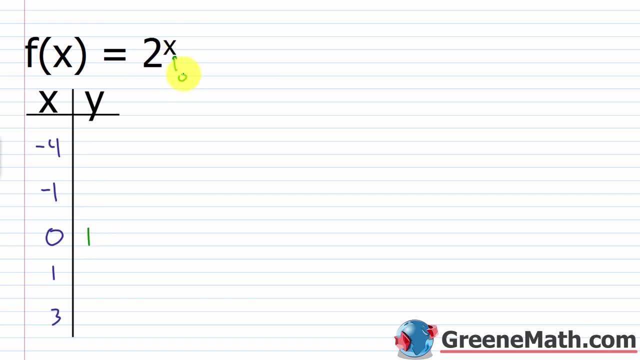 1. If I plugged in a 0 for x there, 2 to the power of 0, by rule is 1.. So f of x or y would be 1.. Now if we look at the other ones, we say y instead of f of x is equal to 2 to the power of. 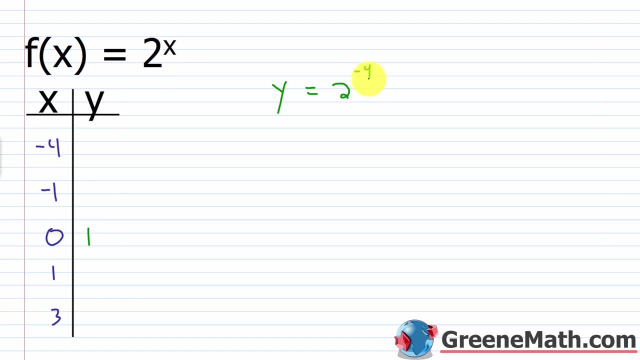 in this case x is negative 4.. So if I plugged in a negative 4 for x, 2 to the power of negative 4 is what This is: 1 over 2 to the fourth power, which is 1 over 16.. So we'll say this is 1, 16th here, And then the next scenario is negative 1.. 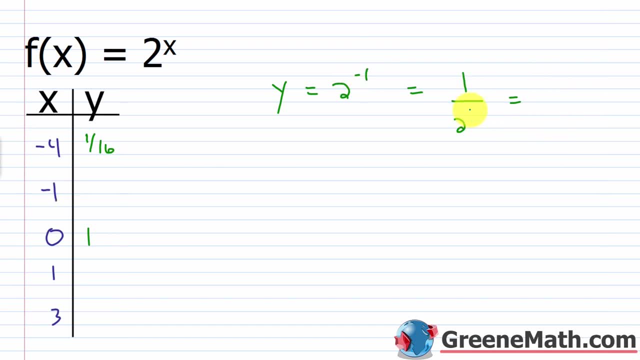 So we know that if we had a negative 1 there, it would be 1 over 2 to the power of 1, which is just 1 half. So this guy would be 1 half. We've already figured this one out. That's 0. 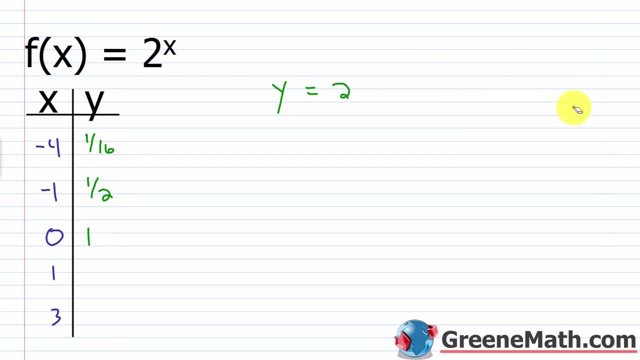 comma 1.. So now we're dealing with positive exponents. So the first one, that's easy: 2 to the first power is just 2.. And then the next one. if we raise this to the third power or we cubed it, 2 cubed would be 8.. All right, So our ordered pairs. here we know we'd 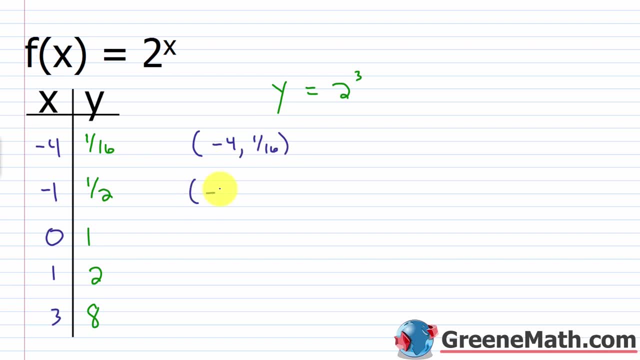 have negative 4 comma 1 16th. We know we'd have negative 1 comma 1 half, We know we'd have 0 comma 1.. We know we'd have 1 comma 2.. And we know we'd have 3 comma 8.. So let's copy these, Okay? So the 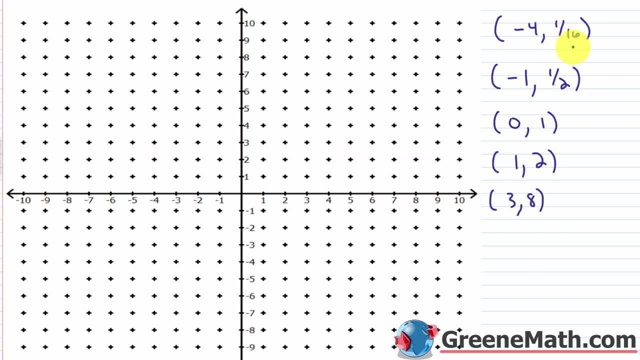 first ordered pair is negative. 4 comma 1- 16th. Now, the way this coordinate plane is drawn, the scale is in increments of 1. So obviously I can't accurately portray 1- 16th. I just have to. 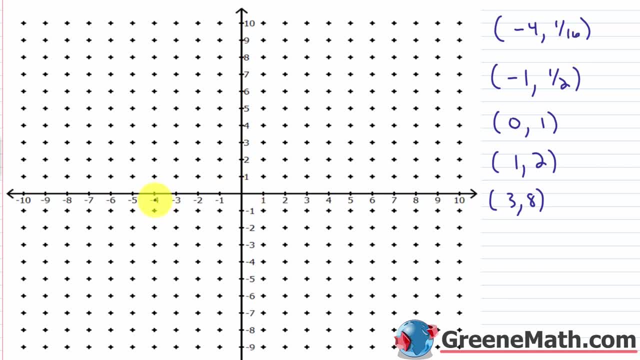 kind of guess at it. So if I go to negative 4 in the x-axis, that's here 1, 16th, let's just say it's about right there. Okay, We're just showing a picture. Again, it doesn't have to be 100%. 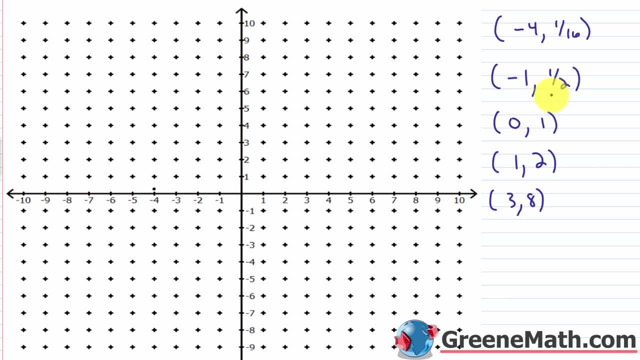 accurate, Then the next point we're looking at is negative 1 comma 1 half. So negative 1 on the x-axis and then 1 half on the y-axis. So it's about right there. Then we have 0 comma 1. So 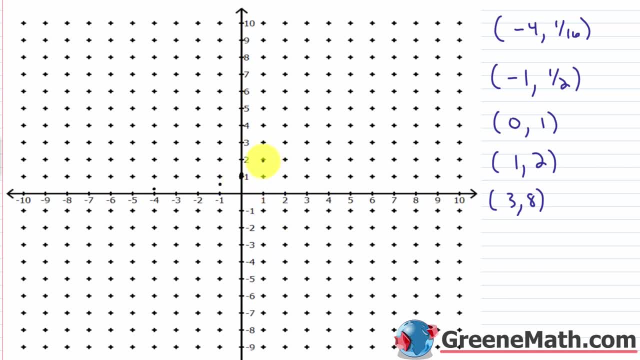 that's about right there. Then we have 1 comma 2. So that's about right there. And then we have 3 comma 8. So that's going to be 3 units to the right, 8 units up. That's about right there. And 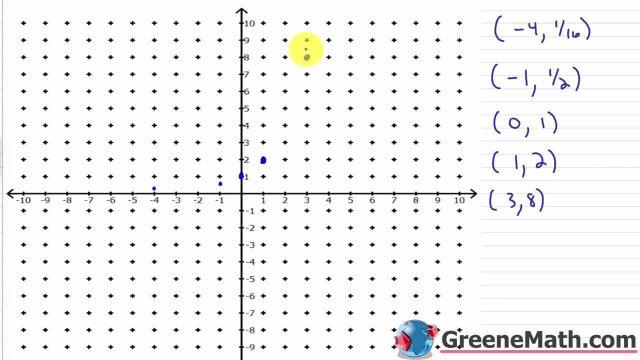 let me kind of go over these with a different color, All right. So as you go to the left here, as these numbers become bigger negative values, what happens is if we go back and look at this guy, you have 2 to the power of something. If I have a really big negative, 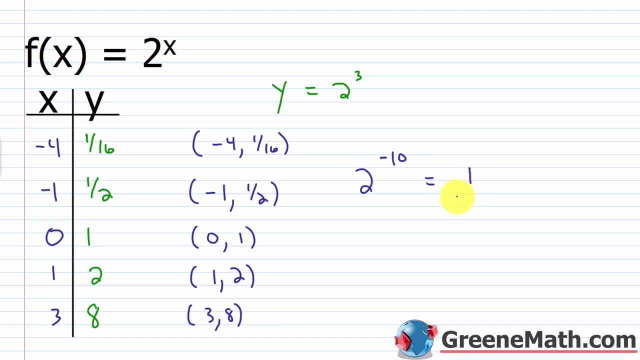 let's say it's 2 to the power of negative 10.. Well, this is 1 over 2 to the 10th power. So as this number gets bigger and bigger, the denominator will get bigger and bigger. So the 1 is divided by a bigger and bigger number, So it becomes a smaller number overall: 2 to the 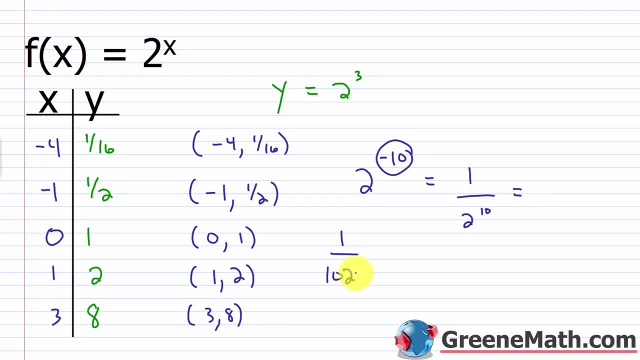 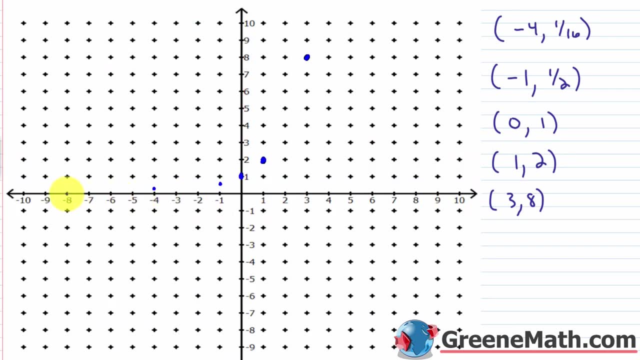 10th power is 1,024.. So you can say I have 1 over 1,024.. This is a small number, right? It's close to 0.. So as you choose bigger and bigger numbers in the negative realm for x, so if I chose negative, 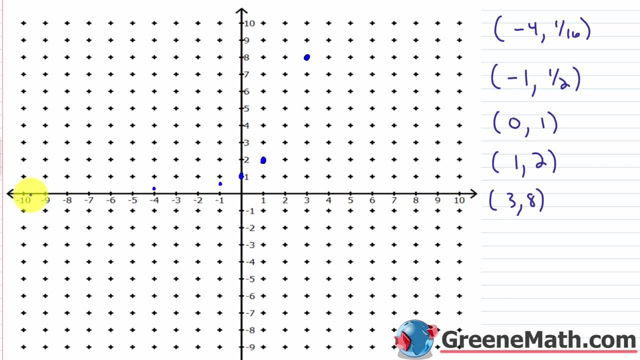 1 million negative, 1 billion negative, 2 trillion, something like that. you're getting the result for y or the f of x value very, very close to 0, because it's a very, very small number. It'll never be 0 and it'll never be negative. So that's why this guy right here, this asymptote, gets formed. 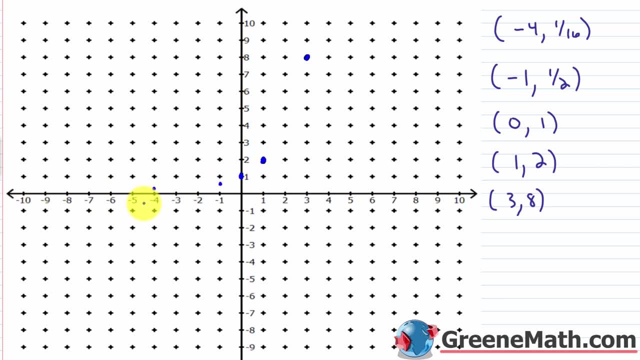 because it's going to approach 0, but it's never going to quite touch it. So what I'm going to do is it approaches the x-axis, a value where y would be 0, but it's never, ever going to actually get. 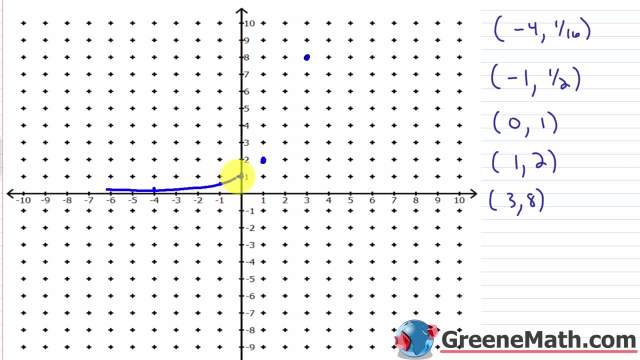 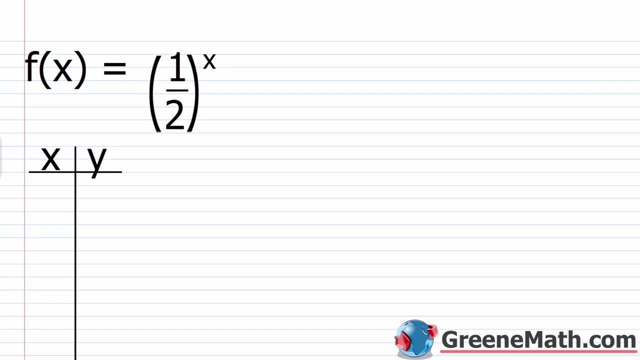 there. So the graph would look something like this: You kind of do like that and then we just hockey stick itself up. We'll do that. Let's take a look at one more of these and then we'll kind of look at some exponential equations. So we have: f of x is equal to one half raised to the power. 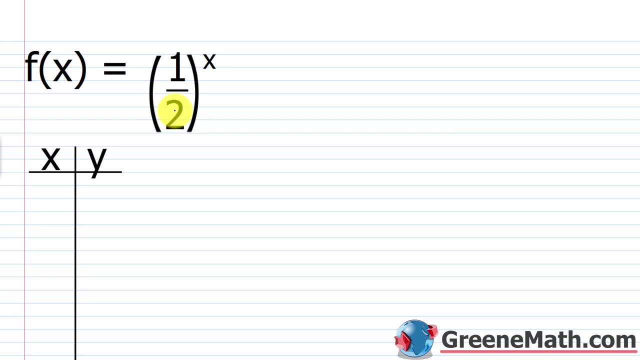 of x. So this guy here is between 0 and 1.. So we would expect the graph to fall from left to right. So we would expect the graph to fall from left to right. So we would expect the graph to fall from left to right. So it's going to start out high and then it's going to come. 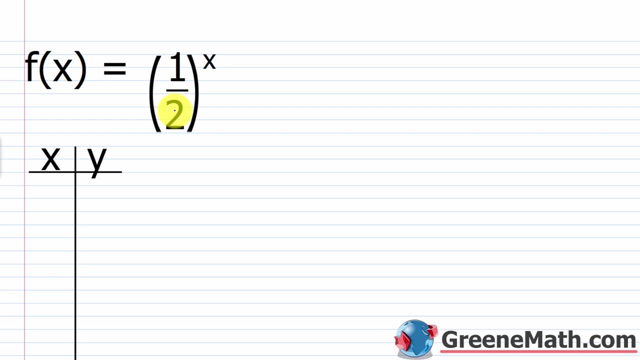 low. It's going to approach the x-axis, but it's never going to touch it. So let's get some points going. Let's do negative 3.. Let's do negative 1.. Let's do 0.. Let's do 1. And let's do 2.. So I know. 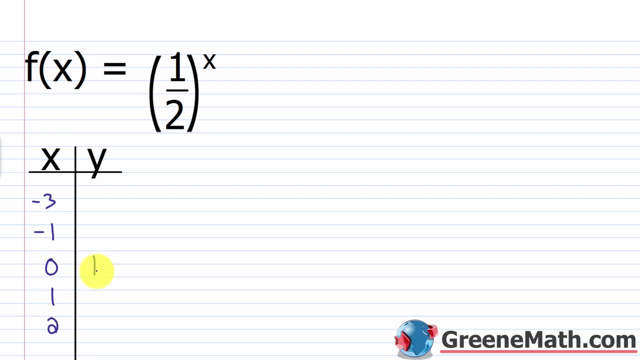 that 0, 1 is a point on this graph. Again, I can always start with that, because I plugged in a 0 there. I know by rule I've got a point on this graph, So I can always start with that because. 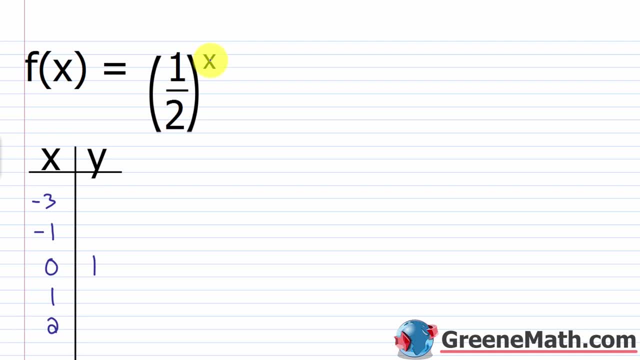 I would get a 1, right. So f of x or y would be 1.. Now let's think about the other ones. I have f of x, or probably be better, just to put: y is equal to one half raised to the power of negative. 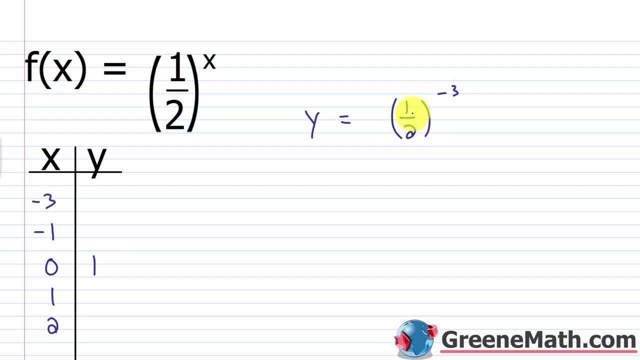 3. So how do I do this? quickly Again, I could flip the fraction here and make that exponent positive. So I could say this is equal to 2 over 1 raised to the power of 3.. So 2 over 1 is just 2.. 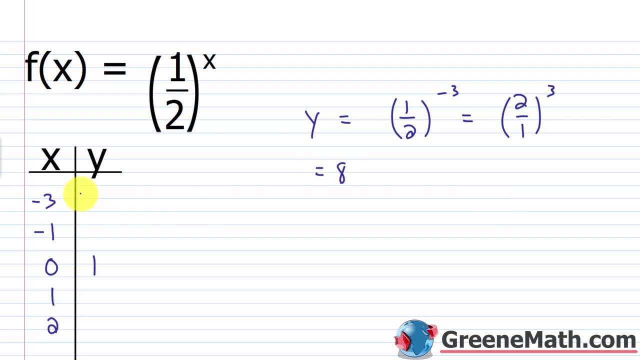 2 cubed is 8.. So negative 3 is x, y is 8.. Now what if x was negative 1?? What if x was negative 1?? We would again flip the fraction, so it would become 2 over 1.. It'll be raised to the first power, So that's just 2.. 0 comma 1,. 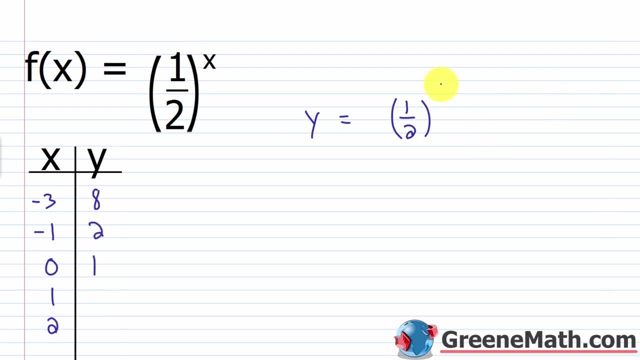 we already have. If x was 1,, y would just be one half. So then, if x was 2, we could say: this is 1 squared, which is 1, over 2 squared, which is 4, or simply 1 fourth. All right, So let's erase this. 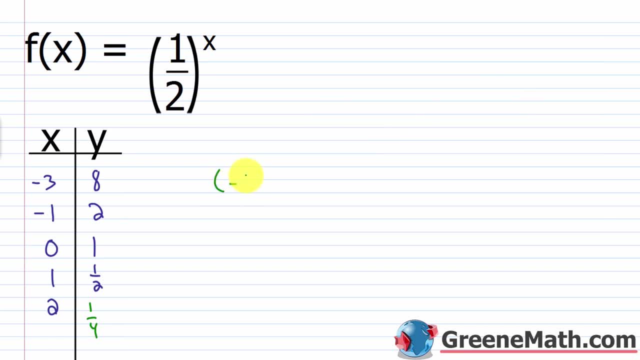 And we'll just kind of jot these ordered pairs down. So we have negative 3 comma 8.. We have negative 1 comma 2.. We have 0 comma 1.. We have 1 comma 1 half And we have 2 comma 1 fourth. So 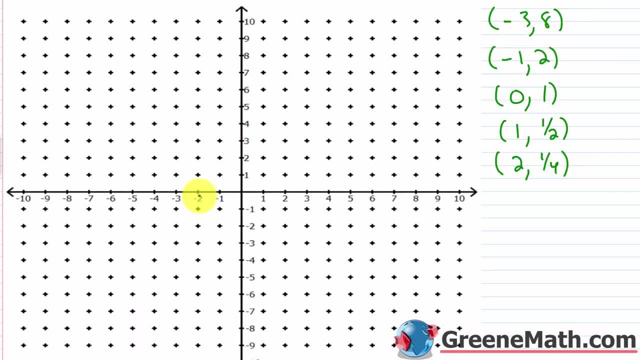 let's just copy this: So negative 3 comma 8.. So negative 3 comma 8, it's going to be right there. Negative 1 comma 2, so that's going to be right there, And 0 comma 1 is right there. 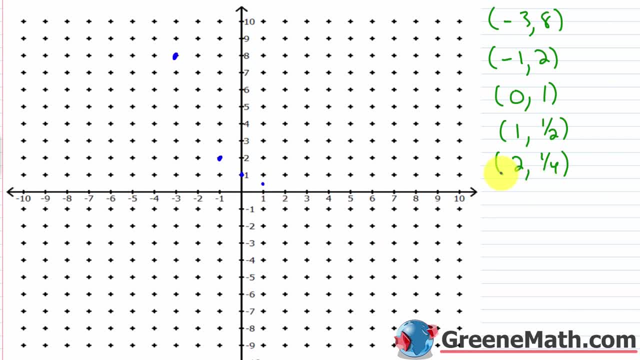 1 comma 1 half will be about right there, And then 2 comma 1 is right there, And then 2 comma 1 is going to be about right there. So you can see, this guy is going to fall from left to right. So 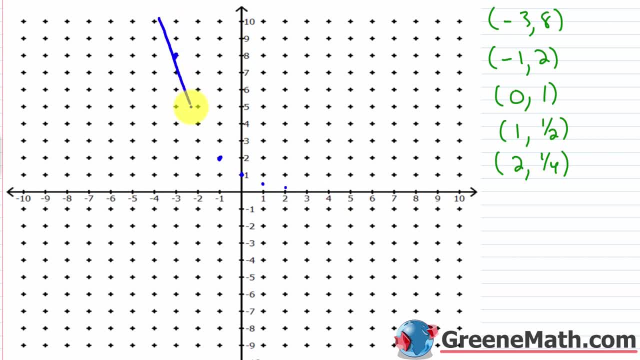 in other words, it's going to come from up here and it's going to fall as we move to the right. So we're going to go that way. We just say that it will again approach the x-axis, but it will never, ever, ever touch it. All right. So now that we've seen what an exponential function. 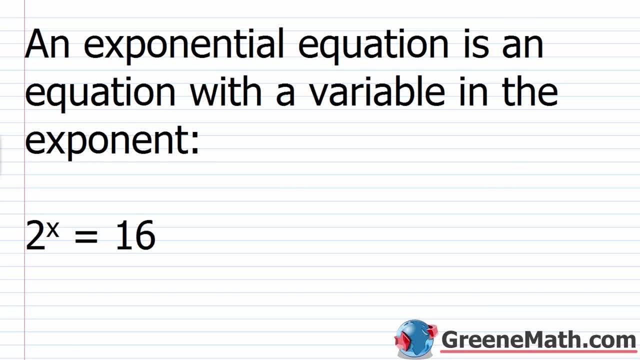 looks like. let's talk about solving exponential equations, And this is mostly what you're going to do. So an exponential equation is just an equation where there's a variable and the exponent. So you see, something like 2 to the power of x equals 16.. Without me explaining how to actually 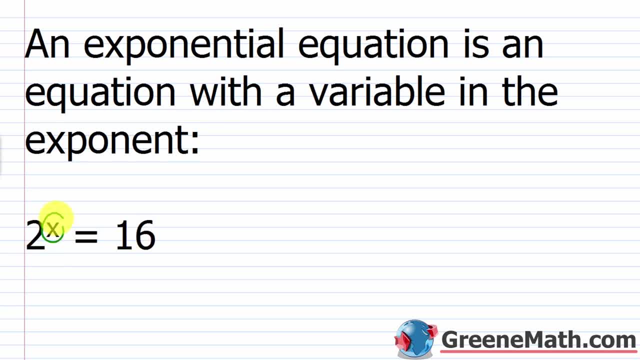 conduct this operation. you could probably guess that x here is equal to 4, right? Just because you know that 2 to the fourth power is 16.. But if you didn't know that off the top of your head, what would you do? So let's talk a little bit about this. So the first thing is just a little 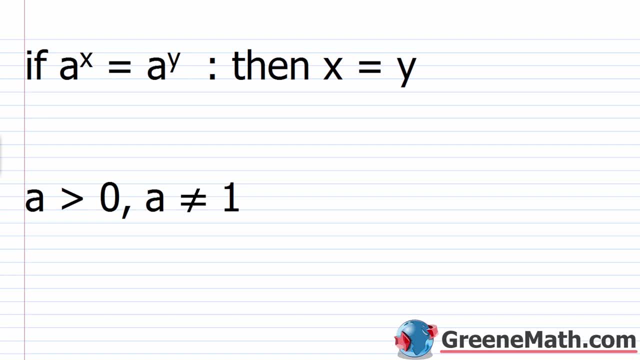 bit of background. So I want you to recall from the last section that a horizontal line test is used to graph the x-axis. So if you're going to do a horizontal line test, you're going to do a graphically determined if we have a one-to-one function. We've already looked at the graphs of 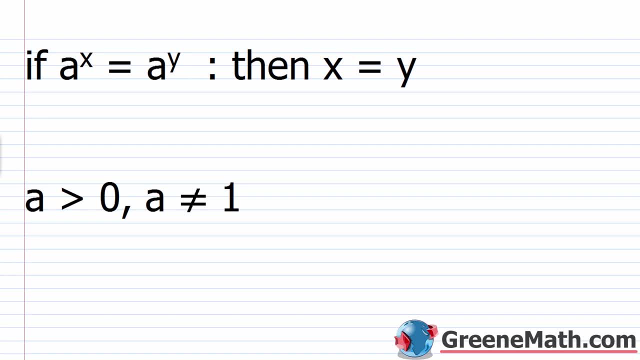 two exponential functions, You could see that a horizontal line would not impact the graph in more than one location. It may seem a little confusing because of that area by the x-axis, But again, if you think about this, you're getting closer and closer to the x-axis. It's never the. 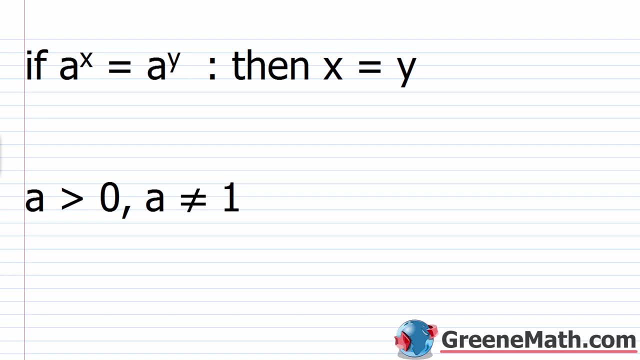 actual same value because it just keeps getting closer, infinitely closer, but it's never actually the same value. So a horizontal line would not impact the graph in more than one location. So it's never actually the same value. So a horizontal line would not impact the graph in. 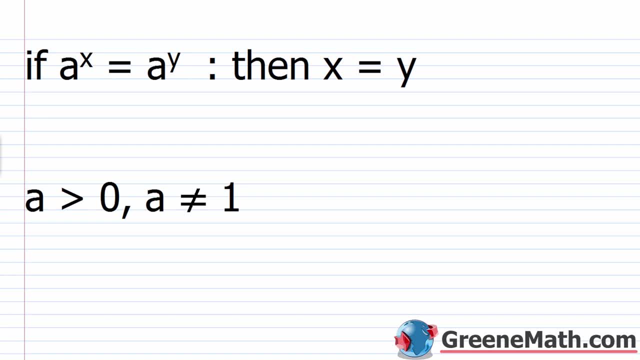 more than one location. So we could say an exponential function is one-to-one. So because of that we can use this kind of rule here. If a is raised to the power of x and this is equal to a raised to the power of y, then we could say x is equal to y. given these restrictions here, that 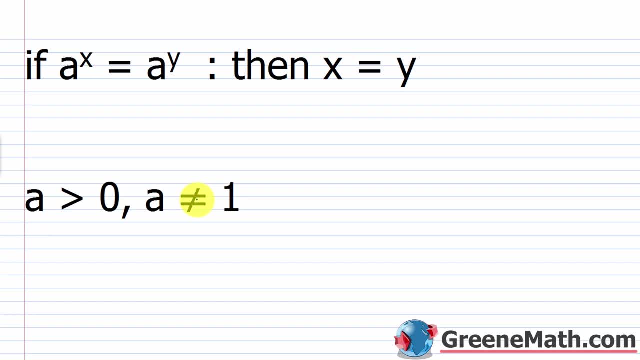 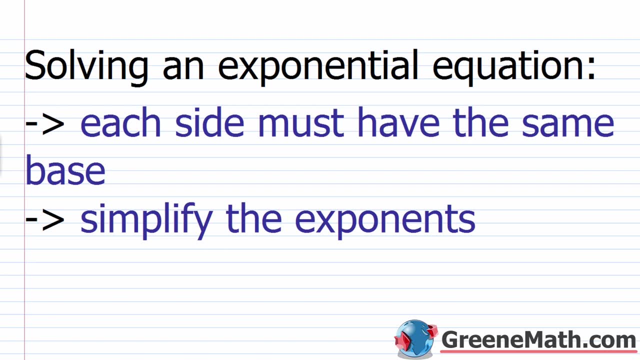 a is greater than zero and a does not equal one. All right, so solving an exponential equation, each side must have the same base. And again that goes back to this rule where we say: if a to the power of x is equal to a to the power of y, the base here is the same. 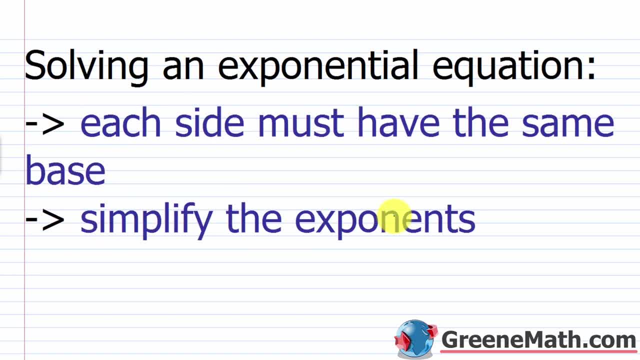 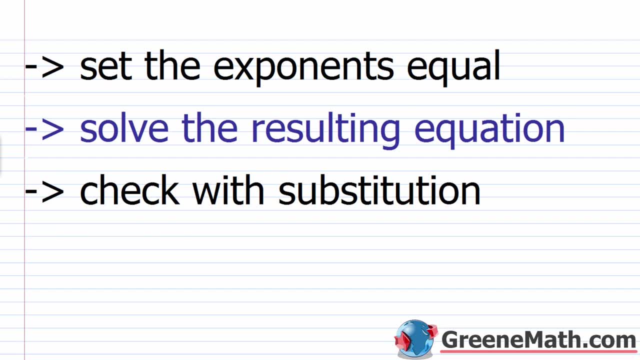 The base is the same. So we say: simplify the exponents. That's the next step. We set the exponents equal to each other, We solve the resulting equation and then we're going to check with substitution. So it's a very, very easy process overall. With the first one we have 2. 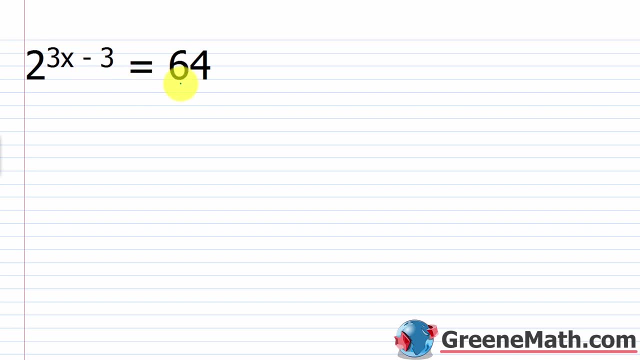 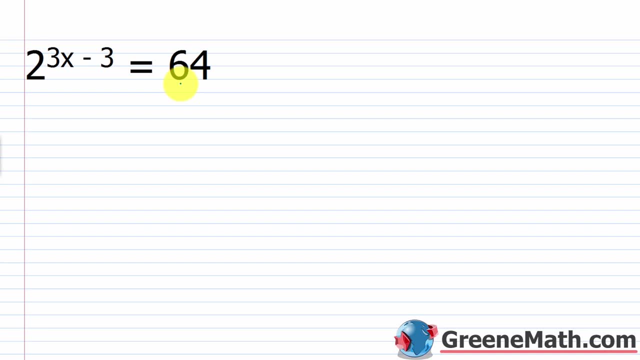 You want to express these as the same base. Well, you know it's 2 to the sixth power. So I would rewrite this and say: this is 2 to the power of 3x minus 3 is equal to 2 to the sixth power. So now, 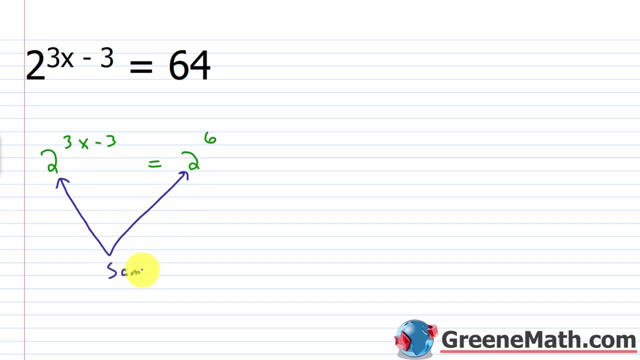 what do I have? I have the same base, Same base. So don't worry about the base, Just take the exponents. So this guy and this guy simplify them and set them equal to each other. 3x minus 3 is: 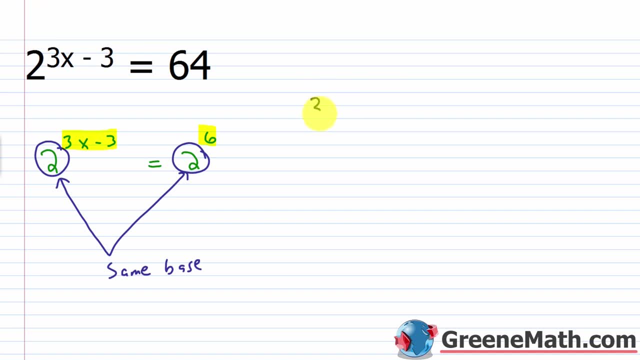 already simplified. 6 is already simplified, So really all I have to do is say 3x minus 3 is equal to 6.. I'm going to solve this very simple linear equation. So add 3 to each side of the equation. 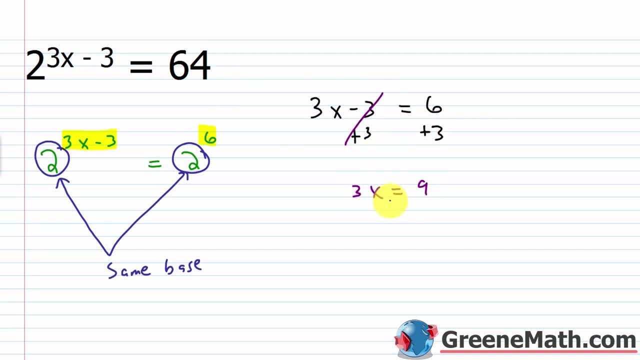 That's going to cancel, I'll have: 3x is equal to 9. Divide both sides by 3. You get x is equal to 3. So the solution set here just contains the element 3. So let's erase all of this. So to: 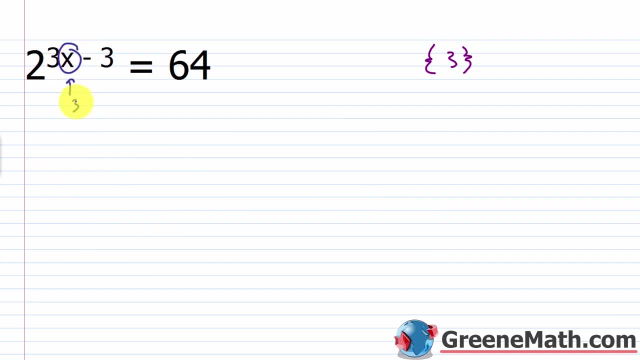 check this. we're going to plug a 3 in for x right there. So you just think about this without even writing anything down: 3 times 3 is what That would give you 9.. Then if I subtracted away 3,, that would give you 6.. So you'd basically have 2 to the. 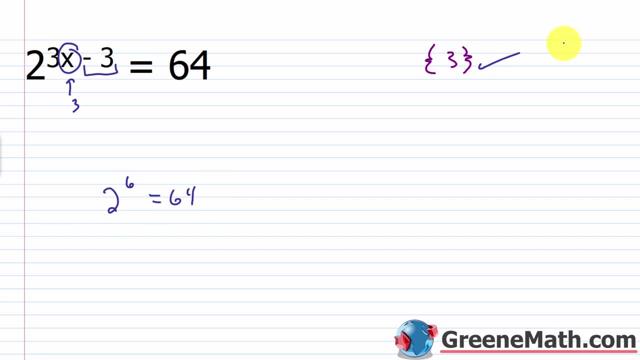 sixth power is equal to 64.. Yeah, we know, that's true. right 2 to the sixth power is 64. You would end up with 64 equals 64. All right, so for the next one, we have 1 ninth raised to the power of. 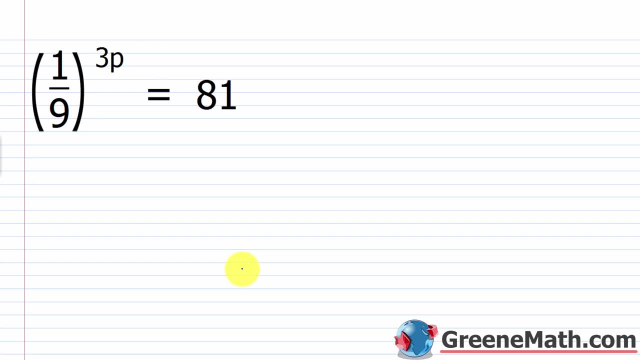 3p is equal to 81. So this one's a little bit more challenging. We just want to think about how to do this, So I'm going to use the same base as 1 ninth. So this is my base, and I want a base of. 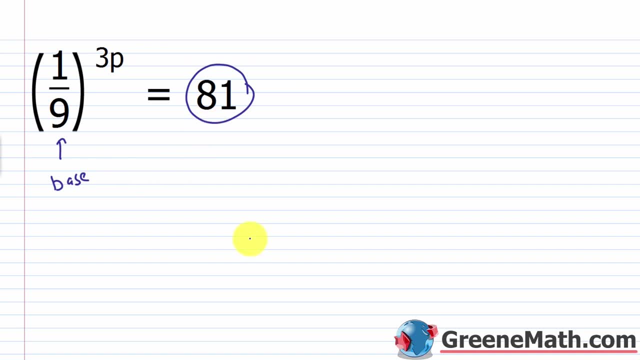 1 ninth. So what can I do? Well, just think about how you could get 1 ninth and change it into 81 just using exponents. Well, I know that 9 squared would give me 81, but that's not going to quite do. 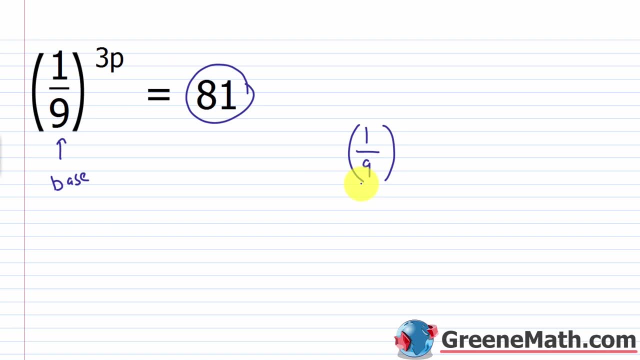 it, because if I square 9 there, I'd have 1 over 81.. So I've got to think about negative exponents. If I use a negative exponent, negative 2 would do the trick right. So 1 ninth raised to the power of negative 2, this would tell me to take the reciprocal of the. 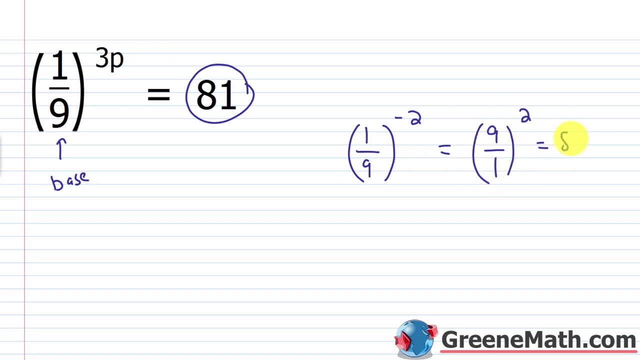 fraction 9 over 1, and square it, which would give me 81.. So this is what I'm looking for here: a base of 1 ninth, an exponent of negative 2.. So let's rewrite the problem to say it's 1 ninth. 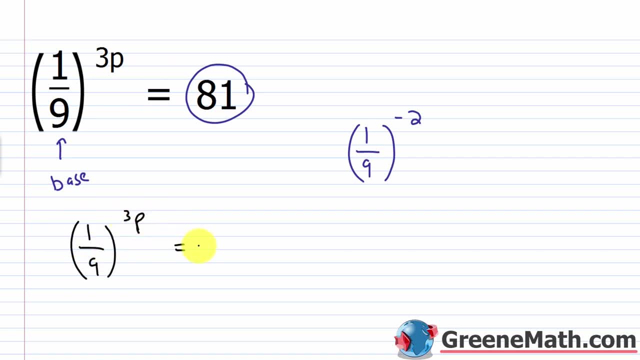 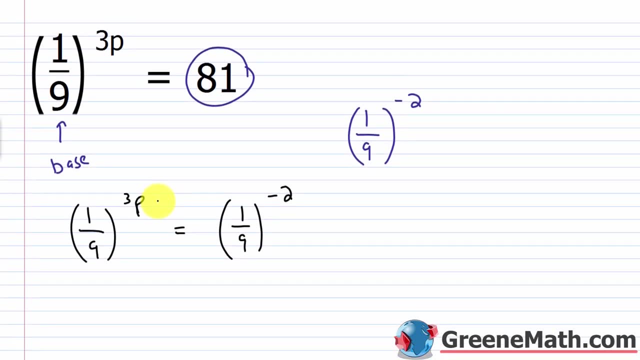 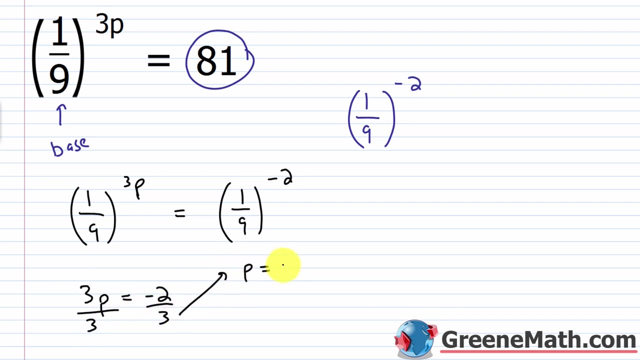 raised to the power of 3p, and this is equal to 1. ninth, raised to the power of negative: 2. The exponents are simplified so I could just set them equal to each other. Let's say 3p is equal to negative. 2. Divide both sides by 3. We'll say that p is equal to negative. 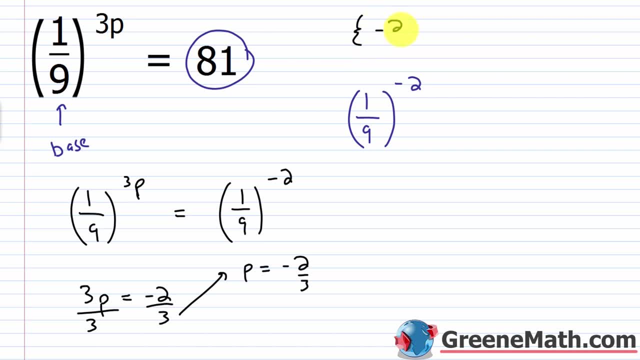 2 thirds. So our solution set here will just contain negative 2 thirds. All right, what about 216? raised to the power of negative 3b minus 2 is equal to 36.. So in this case, if I think about 36,, 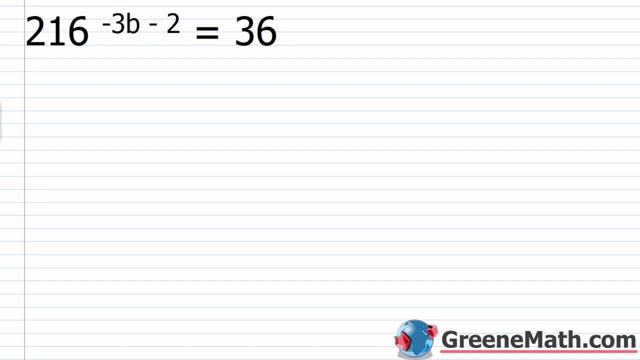 I know that it's 6 squared. If I think about 216, I know that it's 6 cubed, So I want to just write this as 6 squared. I want to write this as 6 cubed, So I think about this just very carefully. 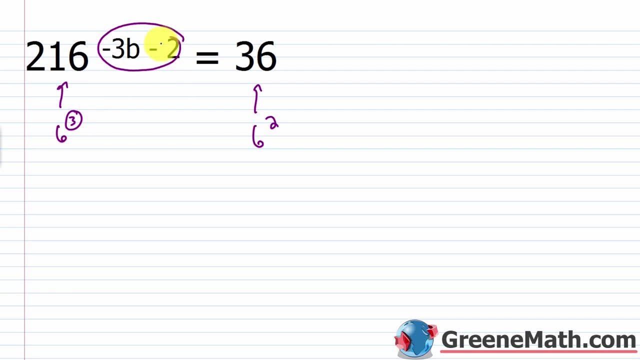 here. This 3 here would just multiply this. So I would have 6 raised to the power of 3 times- in parentheses- negative 3b minus 2. This would be equal to 6 squared. So if I simplify here, 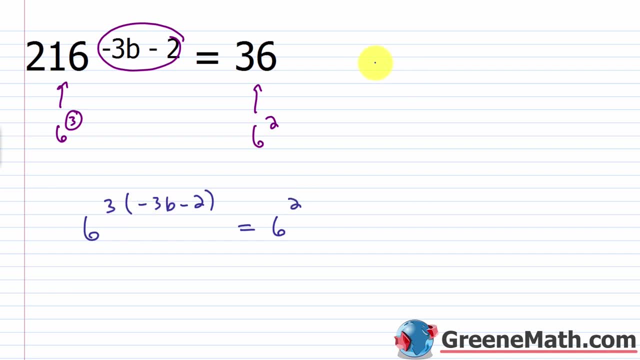 3 times negative 3b is negative 9b, So let's write this over here. We'd have 6 raised to the power of negative 9b, And then 3 times negative 2 would be minus 6. And this equals 6 squared. So I have: 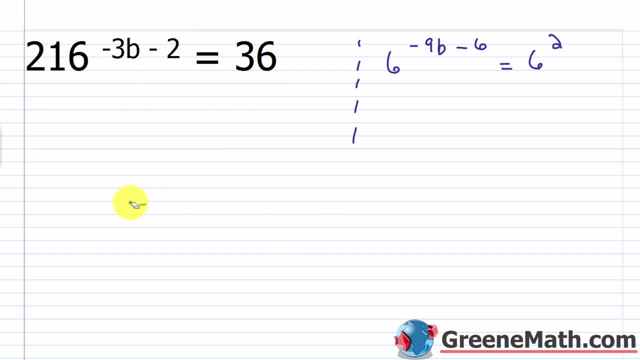 the same base. now All I need to do is take my exponents and set them equal to each other. So, in other words, I will have the equation: negative 9b minus 6 is equal to 2.. I will add 6 to each side. 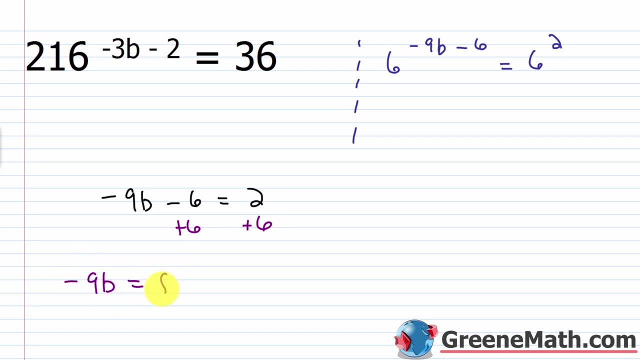 of the equation. That will give me negative 9b is equal to 8.. Divide both sides of the equation by negative 9.. This will give me b is equal to negative 8 ninths. So my solution set here will contain one element, just negative 8. 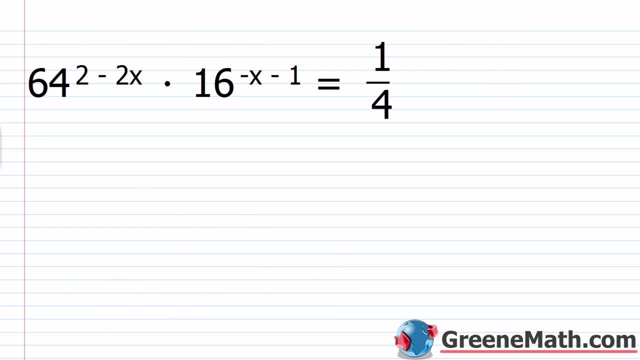 ninths: All right, let's take a look at another one. So we have 64 raised to the power of 2 minus 2x times 16 raised to the power of negative x minus 1.. And this equals 1, 4.. So the first thing. 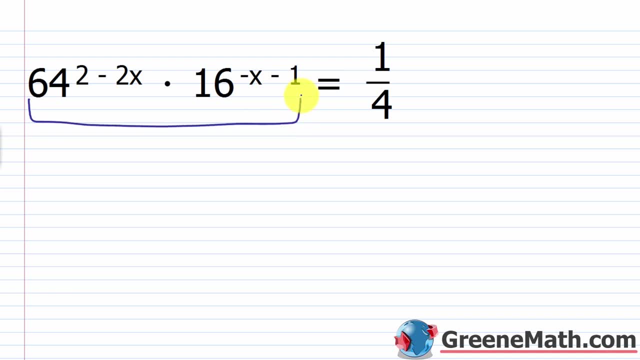 I'm going to do is I'm going to concentrate on simplifying this side. I know that 64 is 2 to the 6th power. I know that 64 is 2 to the 6th power. I know that 64 is 2 to the 6th power. I know that. 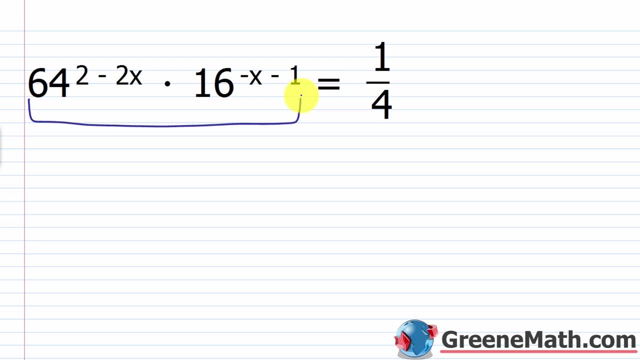 16 is 2 to the 4th power. So let me write these with identical bases. Let's say this is 2 to the 6th power, times this guy right here: 2 minus 2x. that quantity, then times 16, is 2 to the 4th power. 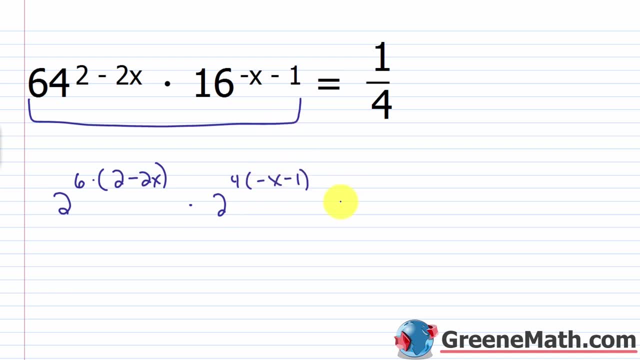 times negative: x minus 1, that quantity And again this equals 1, 4.. All right, so 6 times 2 is 12.. So we would have 2 to the power of 12 minus 6 times 2x is 12x. 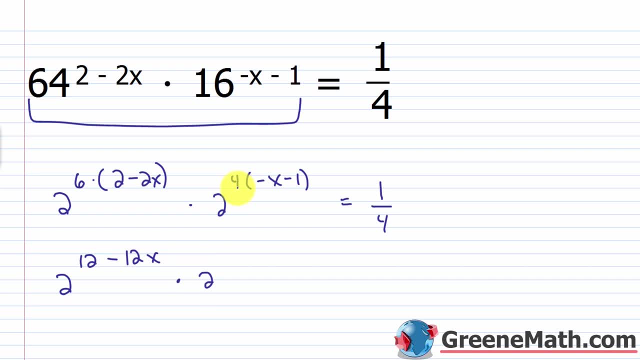 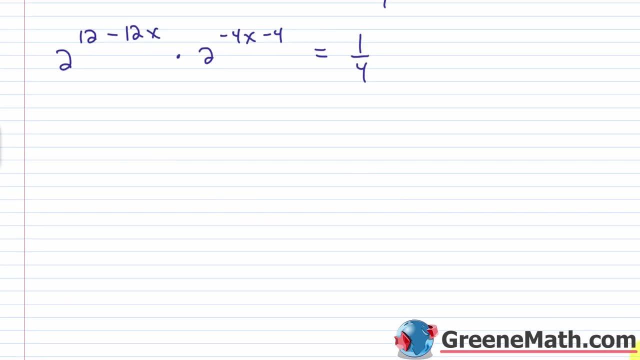 And then times. we have 2 raised to the, we have 4 times negative x. that's negative 4x 4 times negative. 1 is minus 4.. This equals 1- 4th. So now, if we have the same base here, 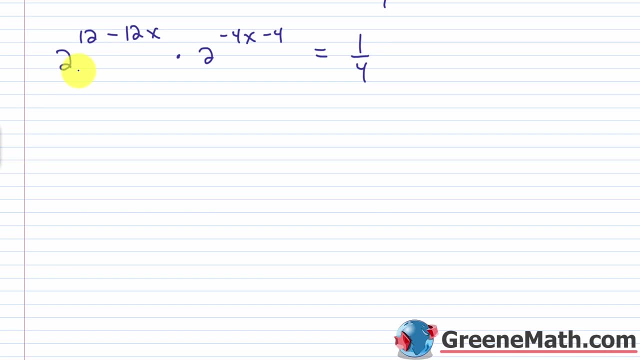 remember, if we're multiplying, we would add exponents. So I could add 12 and negative 4, that would give me 8.. This would be 2 to the power of 8. And then negative 12x minus 4x. 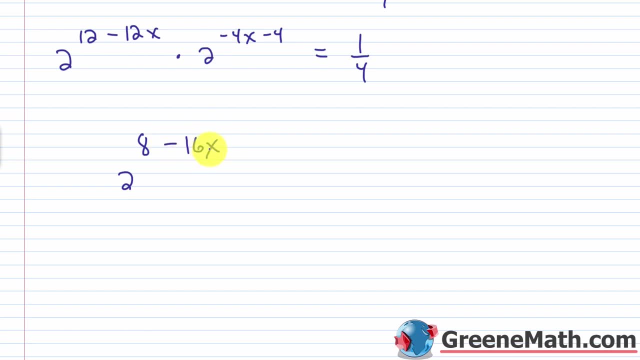 that would be minus 16x, So 2 to the power of 8 minus 16x, and then, if I have this equal to 1, 4th, let's think about how we could rewrite this to have a base of 2.. Well, I could say that 4 is 2 squared, So that's easy enough, but I need 2 to be in the 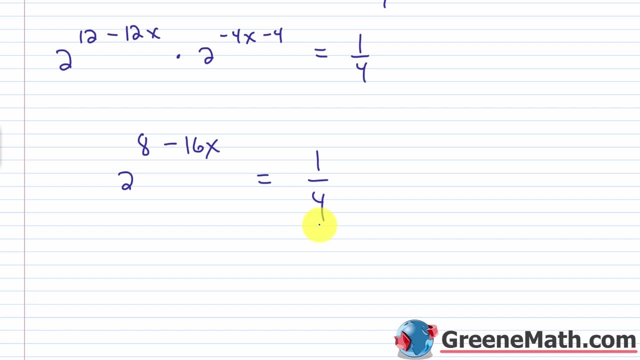 denominator, not the numerator. So I could really rewrite this and say: this is 2 raised to the power of negative, 2, right, Because this is 1 over 2 squared, which is 1- 4th. So let's write this as: 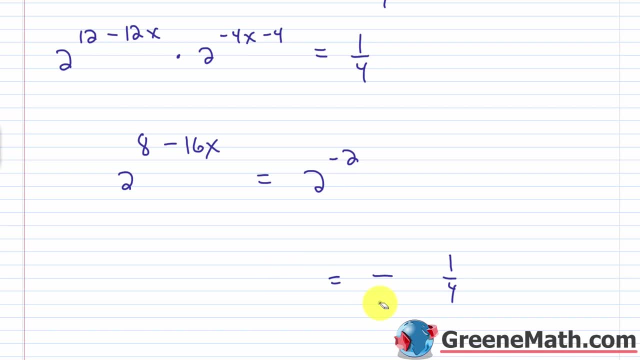 2 raised to the power of negative 2.. And now I'm good to go. I know it seems like a lot of work, It seems kind of tedious, but really, if you know the steps, if you know your rules for exponents, it's not too bad. 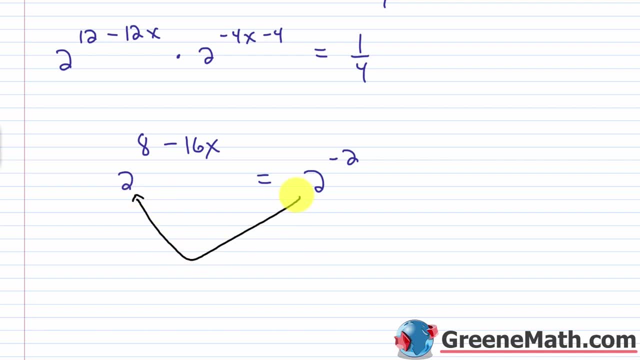 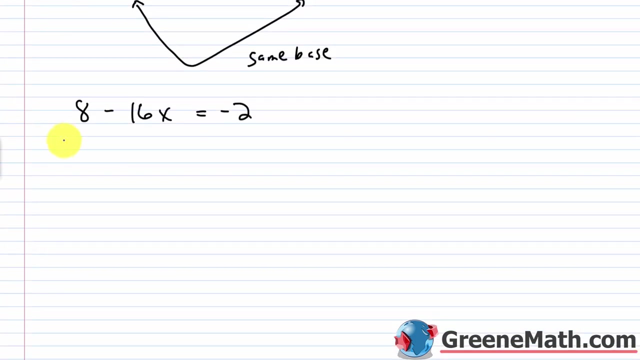 All right, So 2 and 2, same base, same base. I'm just going to set these guys equal to each other. I'll say 8 minus 16x is equal to negative 2, and I'll just solve for x. So I'm going to subtract 8 away from each side of the equation. 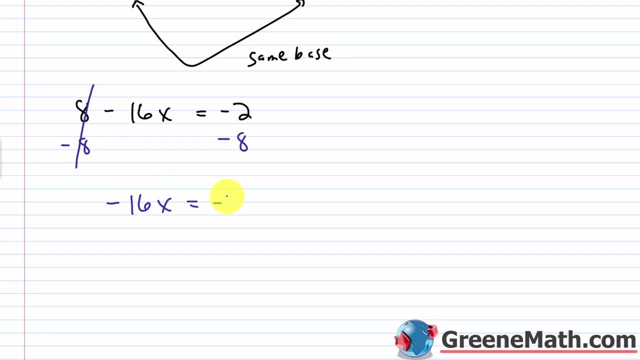 That'll cancel. We'll have negative 16x is equal to negative 10.. We'll divide both sides of the equation by negative 16. And so that's going to cancel. with that, We'll have x is equal to positive. If you think about 10, it's divisible by 2.. Divide it by 2, you get 5.. Divide 16 by 2,. 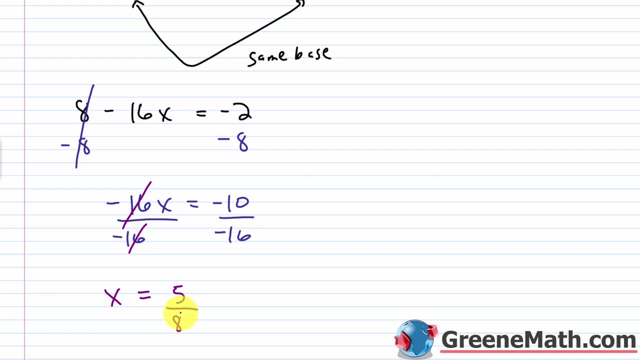 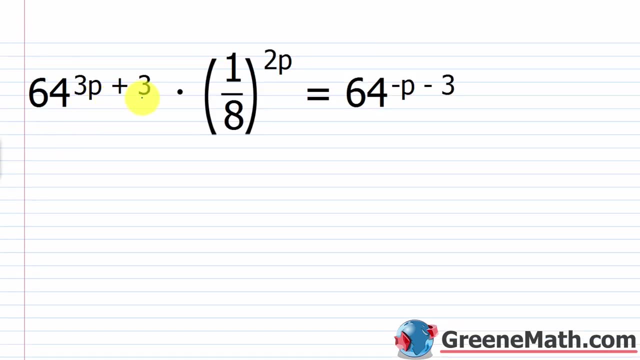 you get 8.. So x equals 5- 8ths. So again, x equals 5- 8ths. All right, So the next problem is 64 raised to the power of 3p plus 3 times 1 8th. So that's going to cancel. with that We'll have: x is equal to. 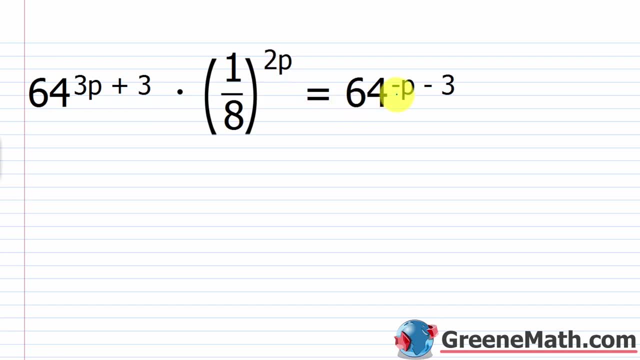 1: 8th raised to the power of 2p. This equals 64 raised to the power of negative p minus 3.. Now we have a 64, a 1 8th and a 64. So let me just use a base of 8.. That would be easy. 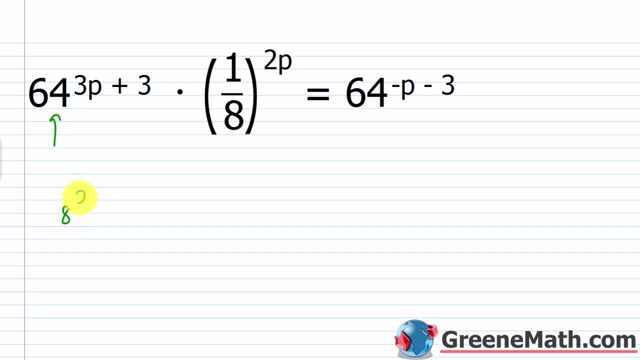 So in other words, I will take 64 and say this is 8 squared And this is multiplied by the quantity 3p plus 3 up here when we talk about the exponents, Then times for 1- 8th. I could really write that. 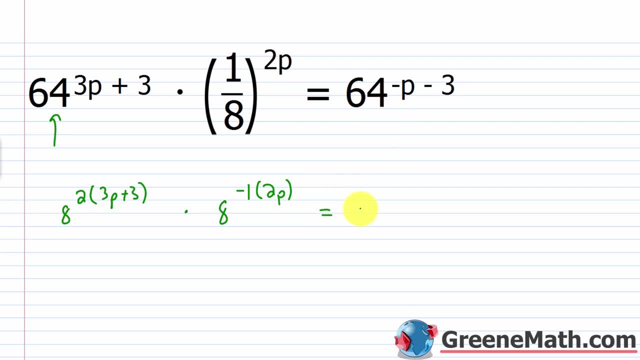 and that's times 2p. This equals for 64. again I could write that as 8 squared And the 2 will be multiplied by the quantity negative p minus 3.. So we'll have 8 and then 2 times 3p is 6p plus 2 times. 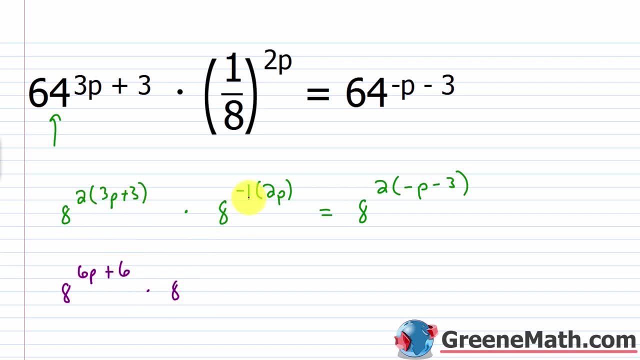 3 is 6.. And then, times 8, raised to the power of negative 1 times 2p, is negative 2p, And this equals 8. raised to the power of 2 times negative, p is negative 2p, And then 2 times negative 3 is. 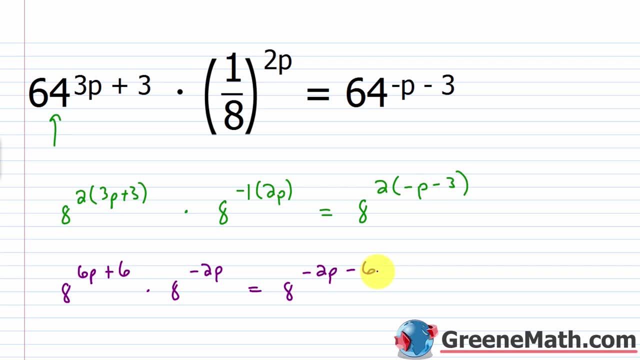 negative 6 or minus 6.. Now we have 8 raised to the power of 2 times negative 2p, And then 2 times negative 3 is negative 6 or minus 6.. 6p plus 6 times 8 raised to the power of negative 2p. If you're multiplying here with the same base, 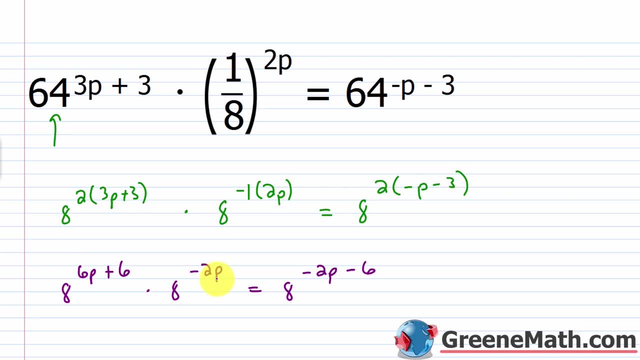 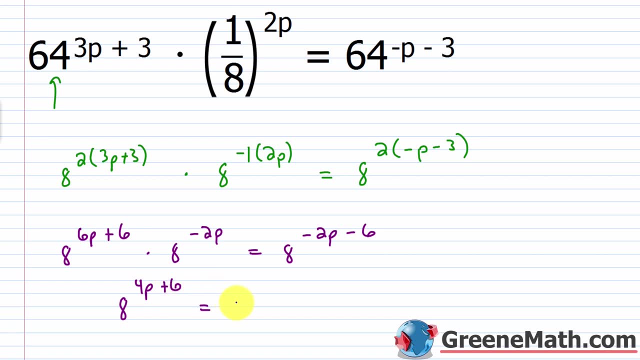 you add the exponents. So in other words I would just add 6p and negative 2p to give me 4p. So this would be 8 raised to the power of 4p plus 6 is equal to 8 raised to the power of negative 2p. 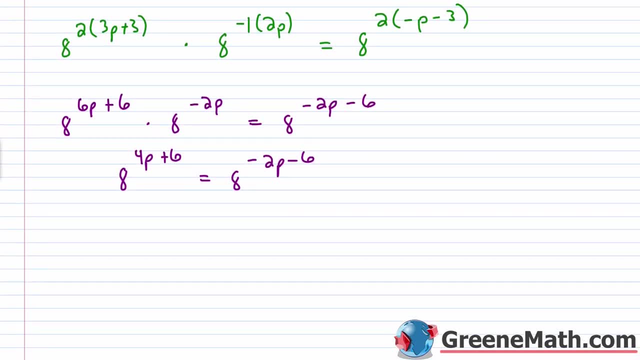 minus 6.. So now we have the same base, So we can just look at the exponents. So we'd have: 4p plus 6 is equal to negative 2p minus 6.. So we have the same base, So we can just look at the. 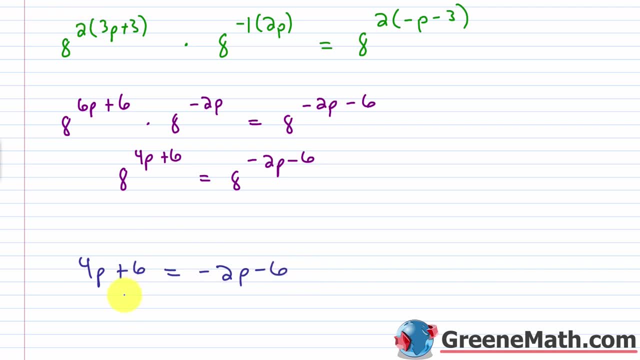 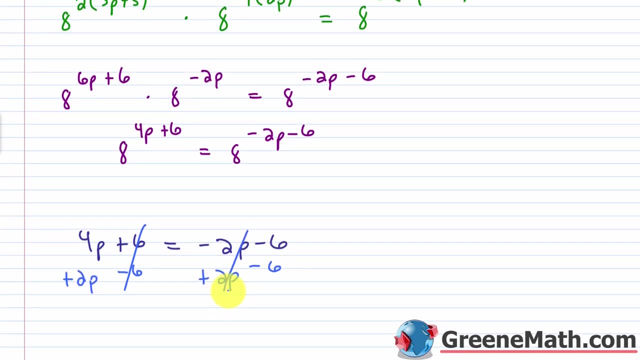 exponents. So we can subtract 6 away from each side of the equation That's gone. We can add 2p to each side of the equation That's gone, So I'll have: 6p is equal to negative, 6 minus 6 is negative. 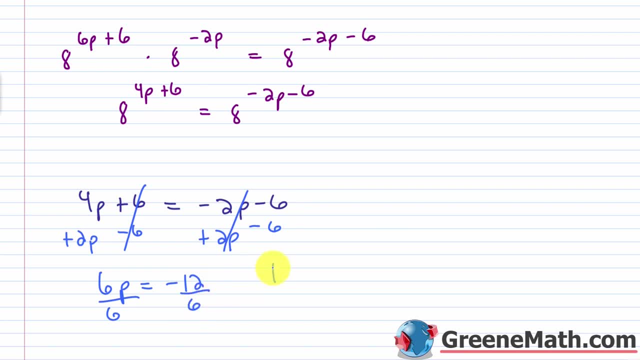 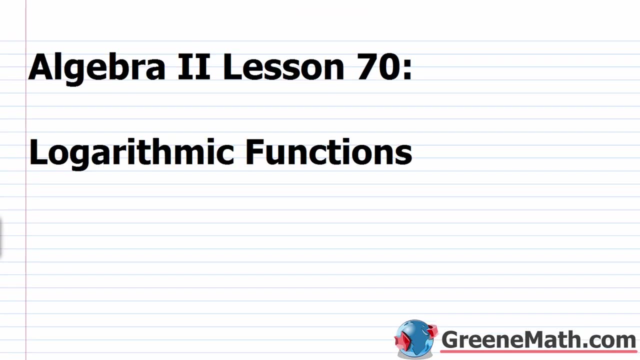 12.. Divide both sides of the equation by 6. We get that p equals negative 2.. All right, let's erase everything. So again, p equals negative 2.. Hello and welcome to Algebra 2, Lesson 70.. In this lesson, 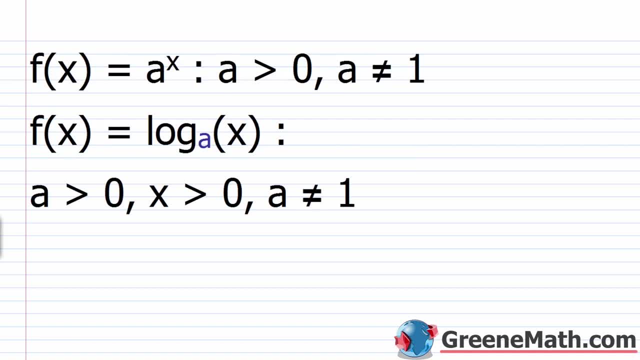 we're going to learn about logarithms. So we're going to learn about logarithms. So we're going to learn about logarithmic functions. So in our last lesson we learned about exponential functions. In that lesson we saw f of x equals. we had our base a raised to our exponent of x. Now 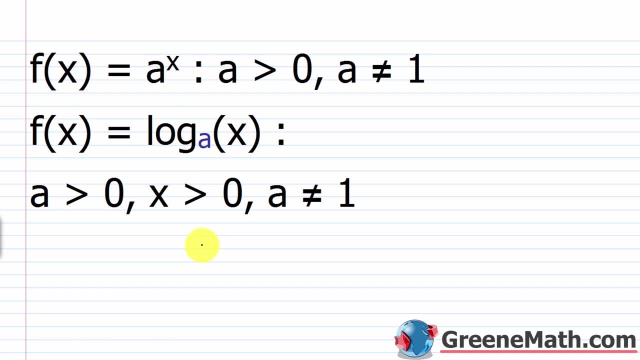 for most of us, this is the first time we ever dealt with a variable in the exponent. As we move forward in math, this is going to be very, very common for us Now. to make everything work, we put some restrictions on the base a. We said a had to be greater than zero. We also said that. 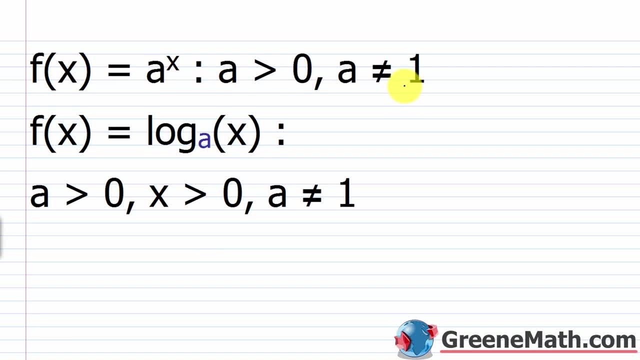 a was not allowed to be equal to the number 1.. Now in this lesson we're going to talk about the inverse of an exponential function. So the inverse of the exponential function is known as the logarithmic function. So the first time you kind of look at a logarithm it may look a little bit. 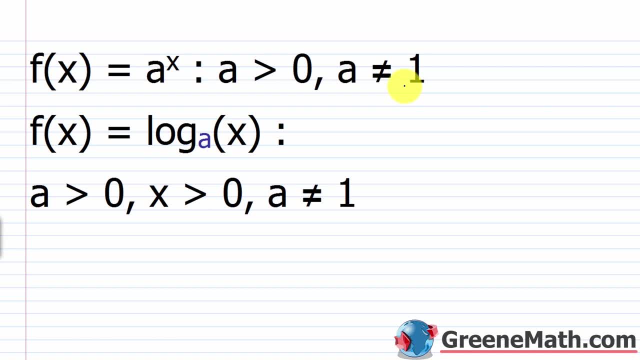 scary to you, right? The notation is very foreign, something you've never come across before. So the first time you read it you'll say f of x equals you have log base a of x, So you're going to have x. So let me kind of write that You'll see log base a of x. Your book might read that a different. 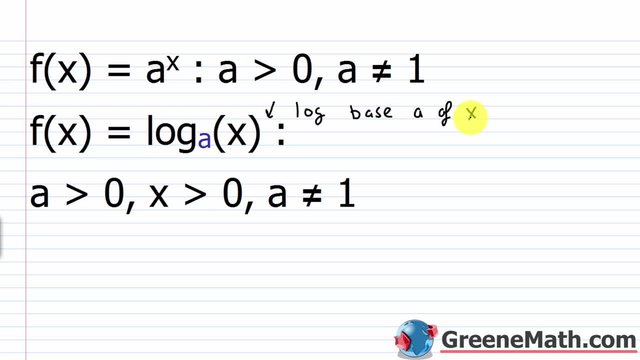 way. Your teacher might tell you a different way. It doesn't really matter, You're conveying the same information either way. Now, in order to make this guy work, we have some restrictions here as well. A, which is referred to as the base. this is referred to as the base. The restrictions are: 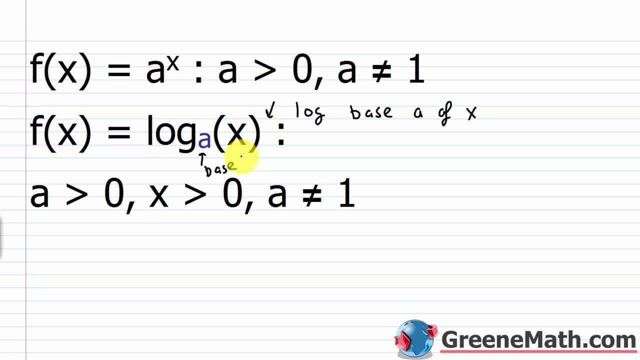 the same as for a And the exponential function. So a has to be greater than zero and a is not allowed to be equal to one. Then x, which is referred to as the argument- Okay, it's called the argument- This has to be greater than zero, And I'll explain why that happens in just a minute. 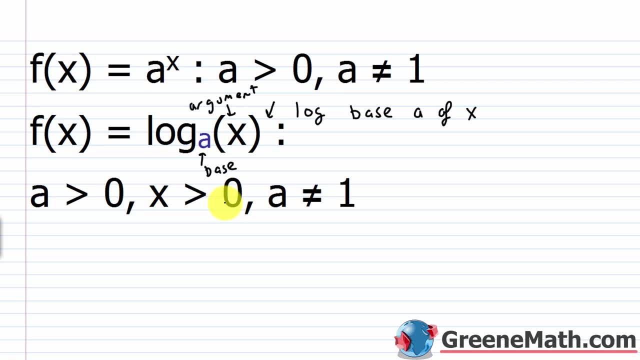 So where does this come from? Well, usually things that are generic come from something. So they're taking this guy right here and then they're finding the inverse of it. So, in other words, if I had let me kind of scroll down, get a little room going. 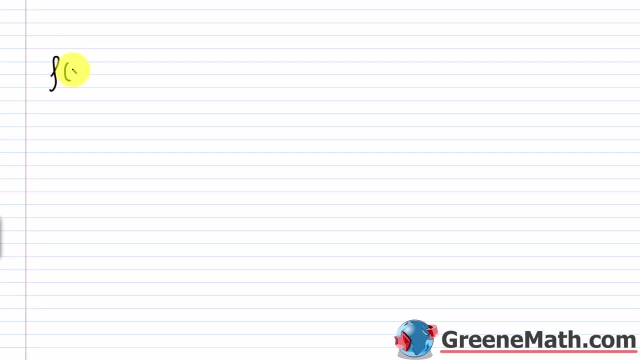 If I had f of x, f of x is equal to a, to the power of x, And again, a is greater than zero and a is not allowed to be equal to one. And I said: find the inverse. Well, the first thing. 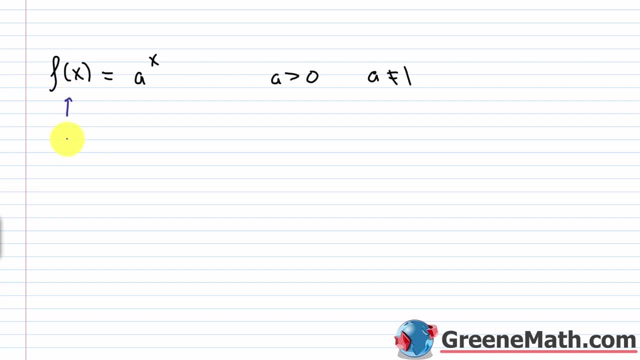 you would do is you would change f of x to y, So this guy would be: y equals a to the power of x. Then you would swap x and y, So in other words, y would become x and y would become y, And then you: 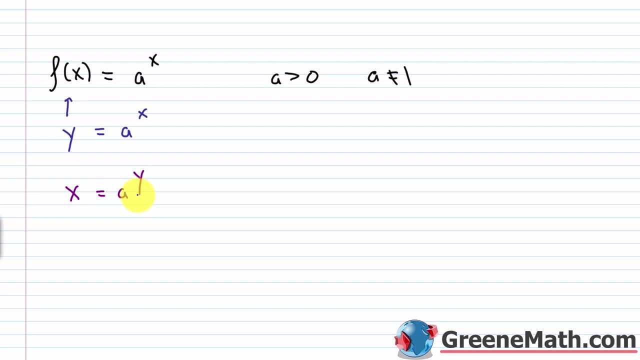 would have: x equals a to the power of y. Now you would solve for y in your next step. But the problem is we have not developed a method to allow us to do that up to this point. So we introduced the logarithm, which allows us to solve for the exponent, or you could say: isolate the. 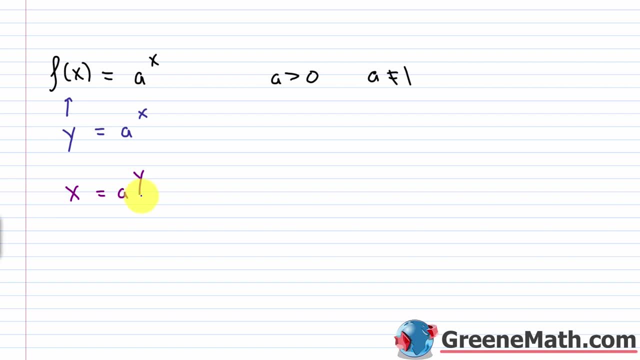 exponent on one side of the equation. So with a logarithm I can say: y is equal to a, to the power of x. So in other words, y is by itself on one side log base a of x. So these two right here. 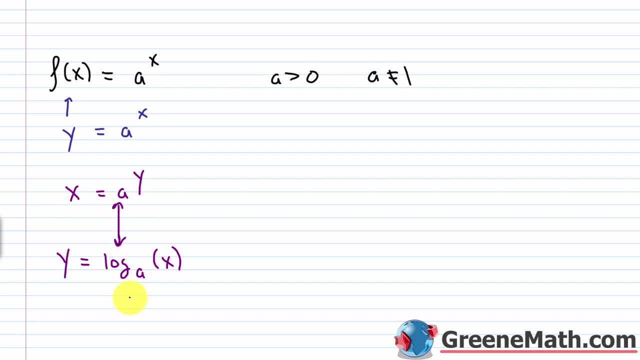 are conveying the same information. This is logarithmic form And this is exponential form, And it's very easy to go back and forth between the two. Now I want to explain why x is going to be greater than zero, So that restriction. 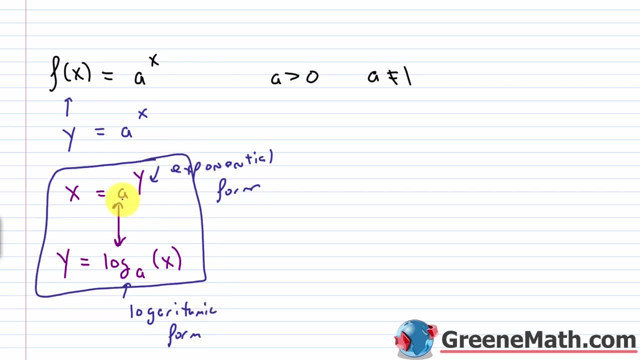 when we get to this part right here, comes from the fact that if I have a and a is greater than zero and a is not allowed to be equal to one, and I raise it to y, it doesn't matter what y is. 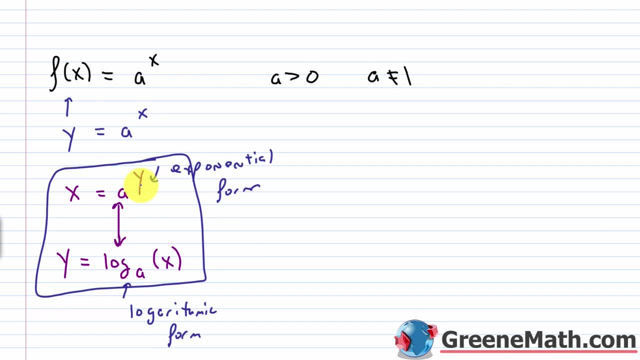 I'm always going to get a result that's greater than zero. Let's say I just pick the number two. If I raise two to some positive number. let's say I do two squared, I get a positive number, So I get four. If I take two and I raise it to some positive number, I get four, So I get four. 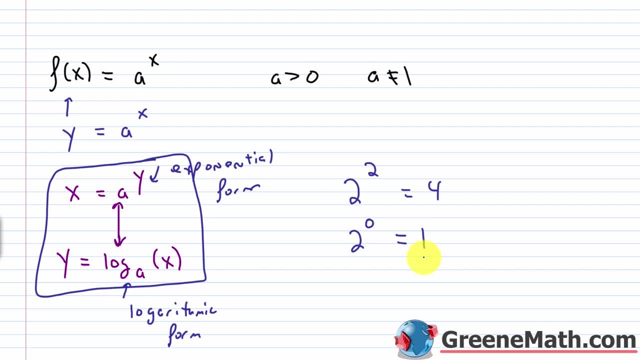 If I raise it to the power of zero, I get one. If I take two and I raise it to a negative- let's say I do negative four- I'm going to get one over two to the fourth power, which is one over 16. This is still positive. It's still greater than zero. So that's why x here. 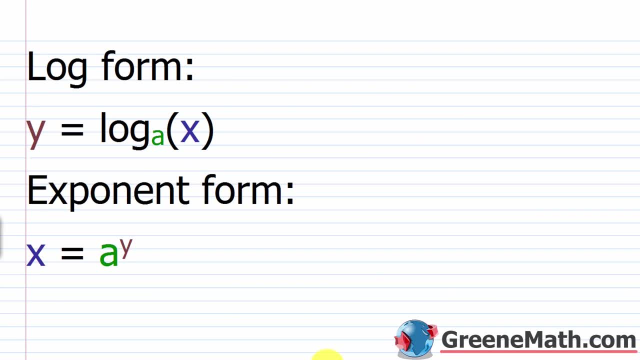 x is greater than zero. All right, so I want to just kind of look at this more cleanly. So we have our log form here, which is: y equals log base a of x. We have our exponent form here, which is: x equals a to the power of y. So we have our exponent form here, which is: x equals a to the power of y. 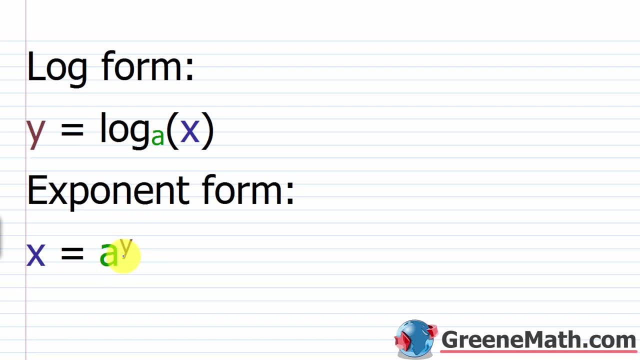 Now we've got to come up with a way to kind of easily send this back and forth between the two forms. Now in your textbook you'll see that a is referred to as the base. A is the base. This is the easy one to remember. The base here is the same as the base here. 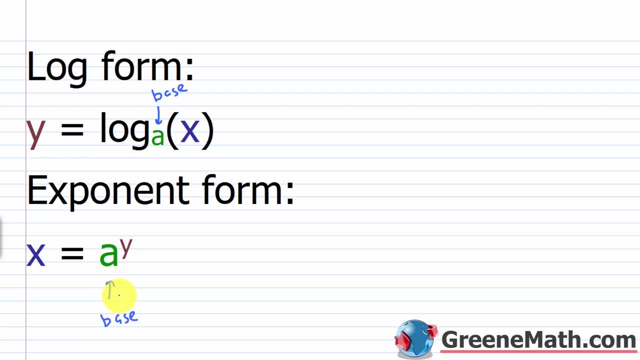 So those two very easy to deal with. Where you kind of get a little bit confused, the technical name for x. when you're looking at it in log form this is referred to as the argument. Sometimes you'll hear it called the power. 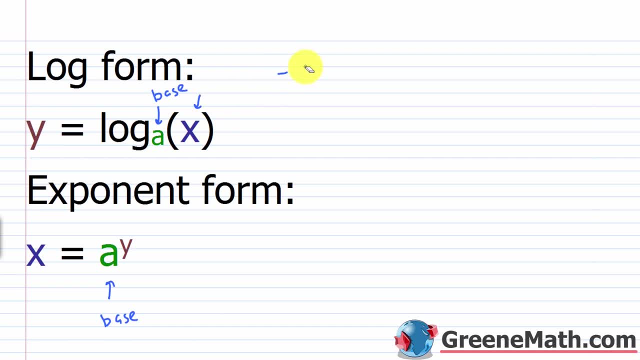 I'm just going to call it the result, And the reason I'm going to do that is just to make it very, very easy to go back and forth. It is the result of taking a to the power of y. So I'm going to say this is the result. You might say it's the answer. whatever you want to do. 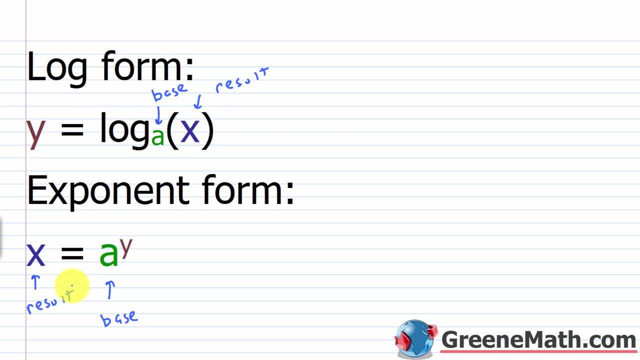 We just need to come up with some easy way to go back and forth between the two, So this works well for my students. Now, y here is the answer in log form, but I'm just going to refer to it as the exponent. 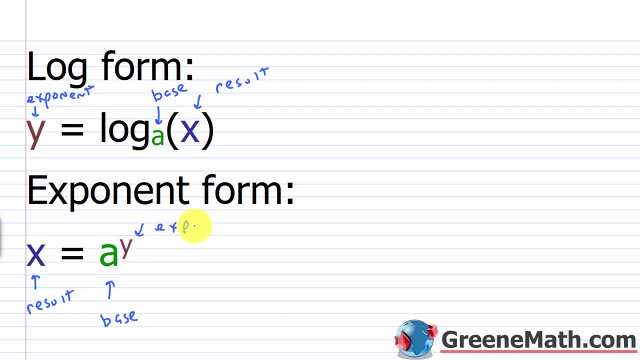 And the reason I'm going to do that is because the exponent here. So I just want to label everything so that we can just go back and forth very easily. So to go back and forth, I know that I would take a, which is my base, I would raise it to my exponent of y and I would get a result of x. 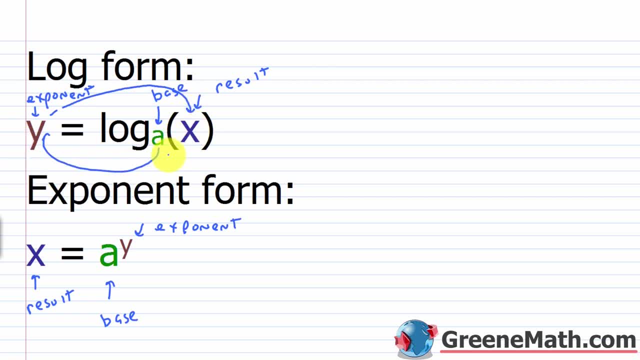 So it's kind of a round robin. You can draw the result of x and you can draw the result of y. You can just go from a to y to x. So if I saw something like two cubed is equal to eight. 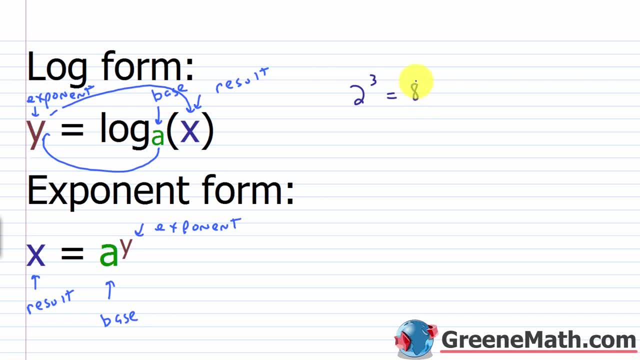 and I said: write this in logarithmic form. you can easily do that. Two is the base, Two is the base, Three is the exponent And eight, we know, is going to be our result. So match that up with what I have here. So I'm going to go back and forth between the two. 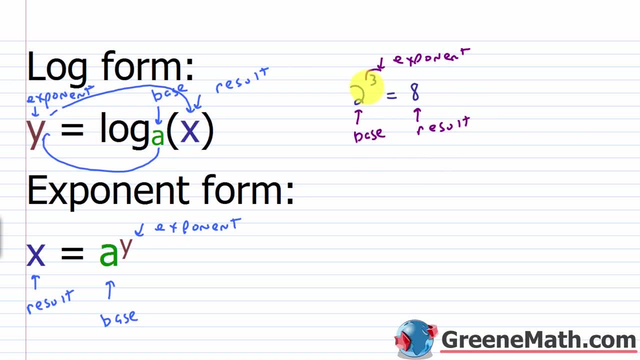 The exponent is by itself. So three will be on one side of the equation by itself. So in other words, it's solved for the exponent. Three is going to be equal to. you have that log word, So just put log and then you have your base. So the base is the same. So two is going to be your. 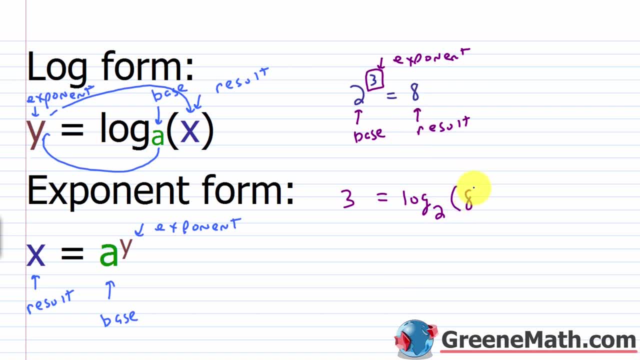 base there And then you put the result, which is eight. Again, the official name for that eight is called the argument, But I'm just calling it the result, so we can keep things consistent and we understand what's going on. So in other words, two to the 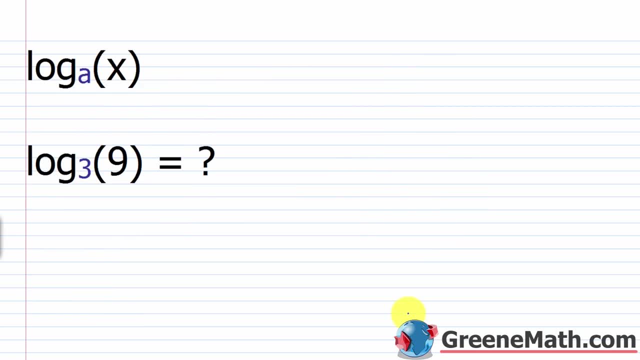 power of three would give me eight, All right. So one thing that might help you is just to realize that log base a of x is just the exponent to which the base a must be raised to to obtain x. I would write that down in my notes or you could write it down with something. 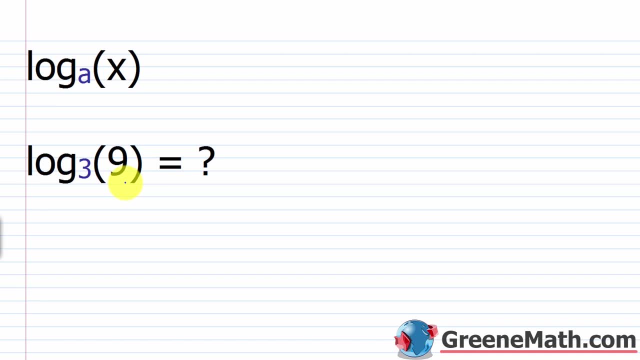 with numerical information in it, So where you can constantly refer to that, So where you can think about the fact that this is just asking me for an exponent, right, It's just asking me to come up with an exponent. So log base three of nine is asking me to come up with an exponent. 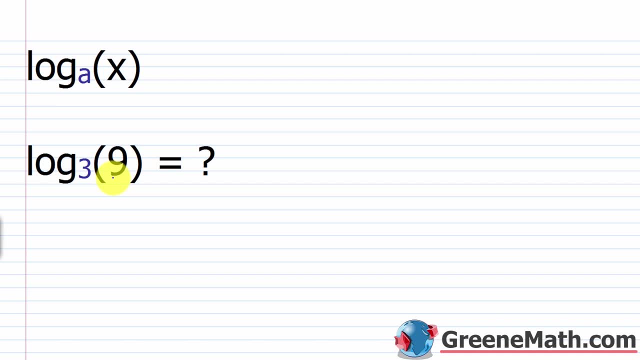 It's asking me: what power does three need to be raised to to obtain nine? In other words, three to the power of question mark equals nine. Three squared equals nine. So this question mark is really just a two. right, I could scratch that out and put a two. So log base three of nine is. 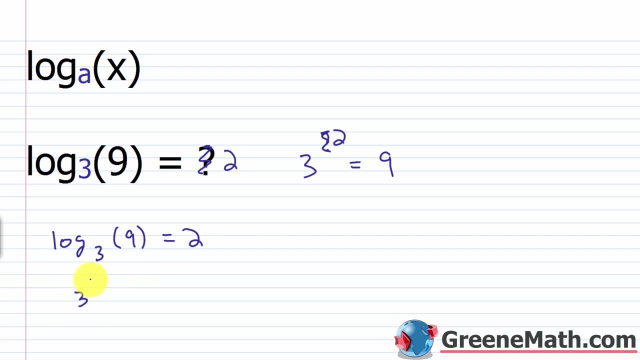 equal to two, or, in exponential form, three squared equals nine. Again, start at the base, go to the exponent and then you put in the exponent: So log base three of nine is equal to 16.. You'll get the result. What about four squared equals 16?? Again, it's solved for the 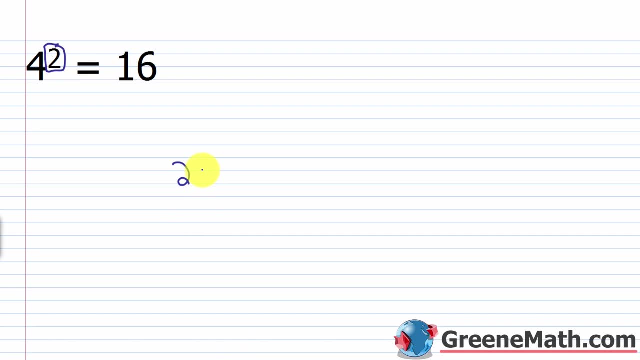 exponent. So two will be on one side of the equation by itself. So two is equal to log. the base is four. So log base four of the result. the result is 16.. So in other words, the base four raised to the power of two would give me the result of 16.. Let's try another one. We have five. 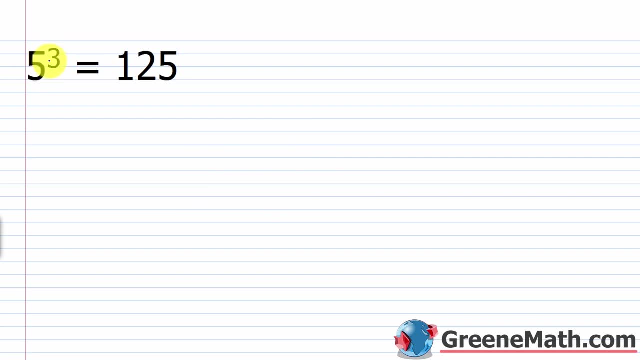 cubed equals 125.. So again, five cubed equals 125.. So again, five cubed equals 125.. So again, five is the base, three is the exponent. 125 would be the result. So I would have three. 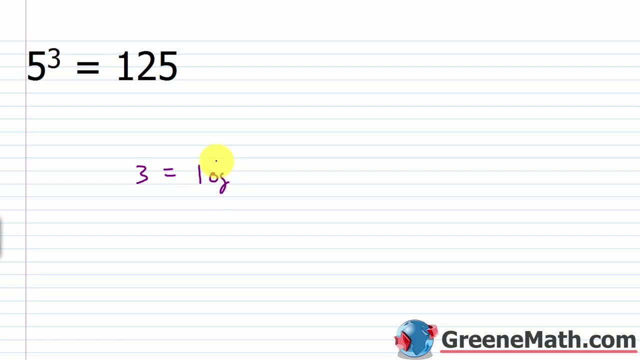 the exponent is equal to log. the base is five. So log base five of our result is 125.. Let's try one more. So we have 10 raised to the power of negative two equals one over 100.. So my exponent is negative two. Negative two is on one side. by itself, This is equal to. you have a log. 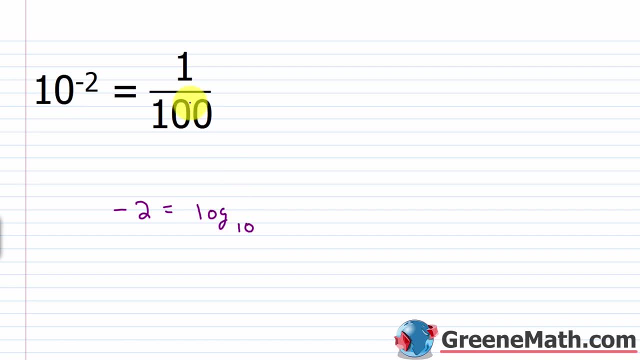 you have a base of 10.. So a base of 10, and then of one over 100.. Now you can again say that 10,, which is our base, raised to the exponent of negative two would get me to a result of one. 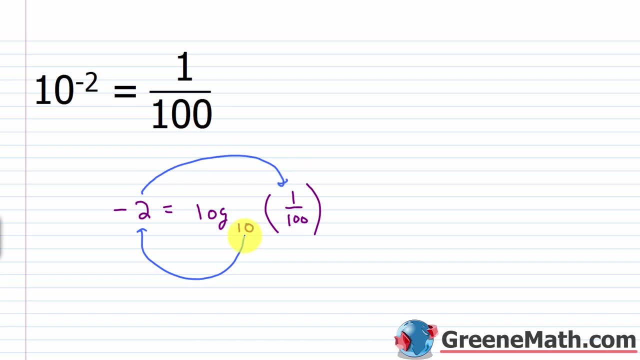 over 100.. We're going to learn later on that if you have a base of 10, you don't need to write. it's called the common logarithm. But we'll see that in a few lessons. All right, so at this point, 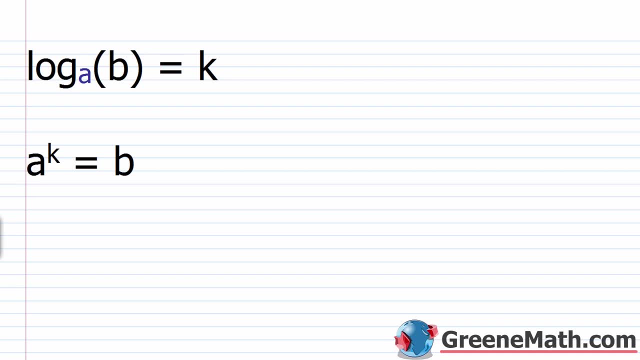 you've seen some examples of a base of 10, and you've seen some examples of a base of 10.. So how to convert between exponential form and logarithmic form? It's really easy. It's just something you need to practice a lot, kind of to get used to it, and then it becomes second nature. 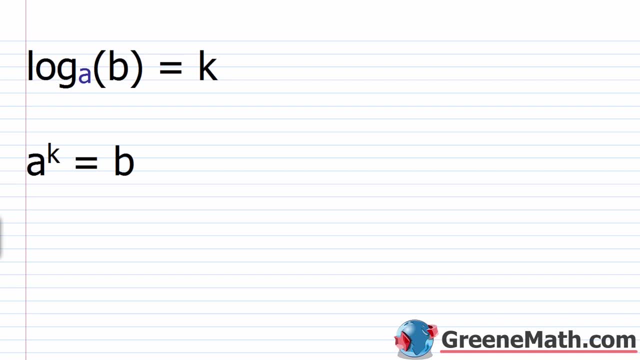 to you. So now we just want to talk about how to solve a simple logarithmic equation. When we get into the next few sections we're going to see that these get much more complicated, But for right now we're going to focus on the easy ones. So if we have log base A of B and we say this is: 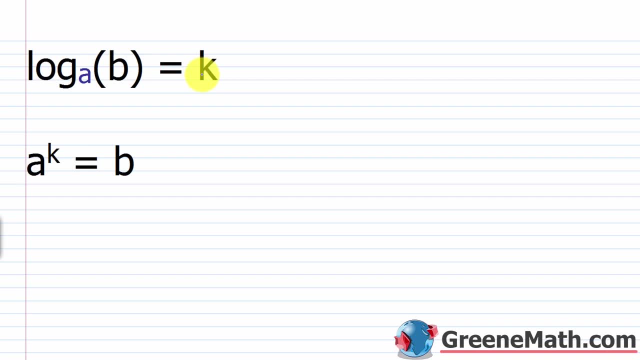 equal to K. we can solve this problem. So we're going to solve this problem. So we're going to do this by putting it in exponential form and just using the rules that we learned in the last section. right, Remember, if you have the same base, you can set the exponents equal to each. 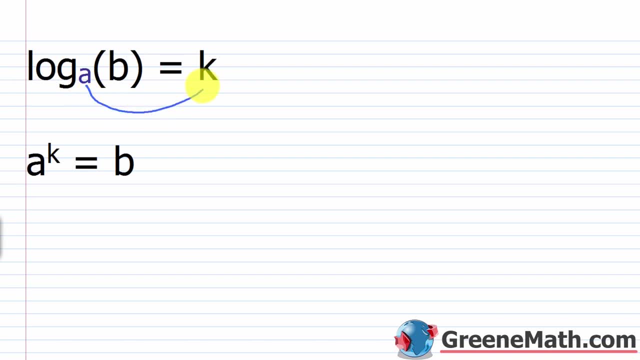 other and you can solve. So here we would say: the base A is raised to K and this is equal to a result of B. So A to the power of K equals B. All right, so for the first example we have, 3 is: 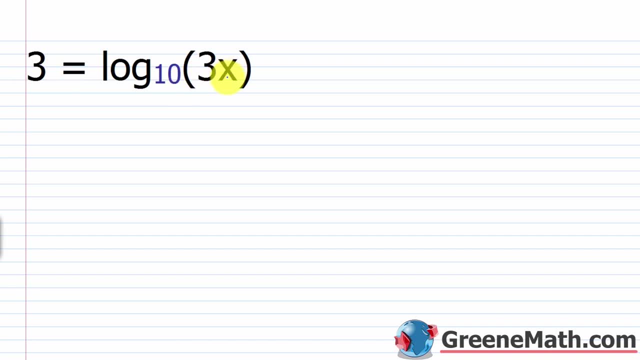 equal to log base 10 of 3x. So 10 is raised to the power of 3.. And this is equal to a result of 3x. So what do I do here? In this particular case? it's pretty easy. We know that 10 cubed is 1,000.. So let's just start with that. So it's a 1 followed by 1,. 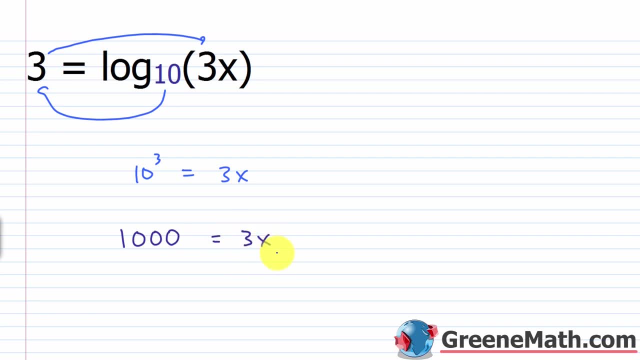 2, 3 zeros, So that equals 3x. If I want to isolate x in this case, I just divide both sides of the equation by 3, and I'll end up with x is equal to 1,000 over 3.. 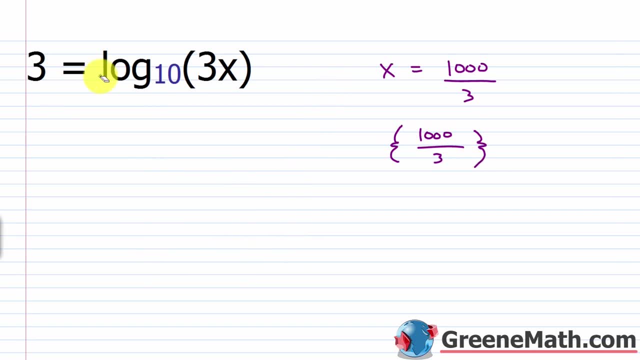 Let's erase this real quick. Checking this guy is super simple. If I plugged in a 1,000 over 3 for x there, what would I have? I would have: 3 is equal to log base 10 of 3 multiplied by 1,000. 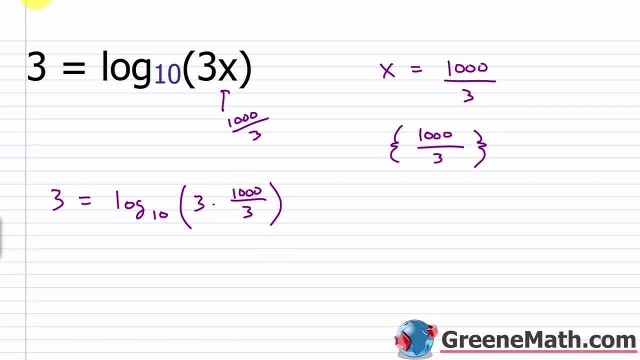 over 3.. And so is this true? Well, this cancels with this and I'm left with 1,000.. So, in other words, is 10 cubed equal to 1,000 over 3?? Well, this cancels with this and I'm left with 1,000. 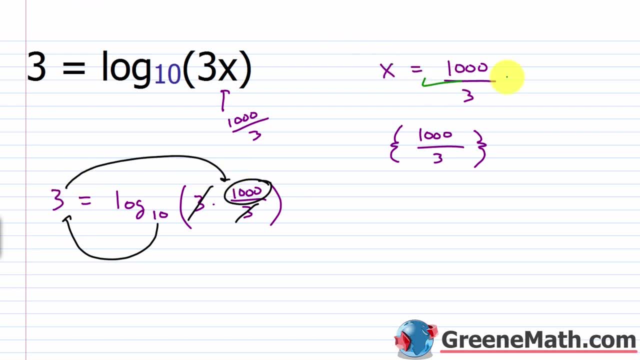 Yes, it is right. So we can check this guy off and say x equals 1,000 over 3 is the correct solution. All right, let's take a look at another one. So we have log base 5 of negative 4x plus 5. 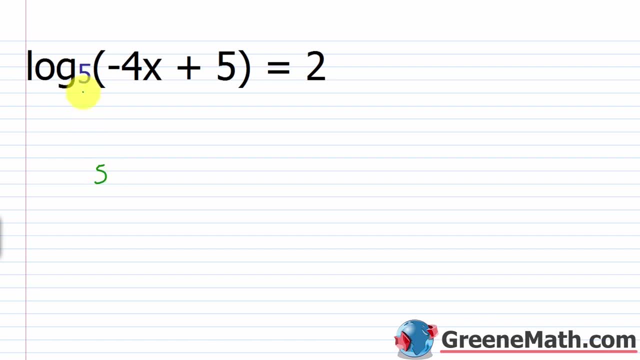 equals 2.. So we'd have 5, which is our base, raised to the exponent of 2.. And this is equal to our result, which is negative 4x plus 5.. So another easy one: we'd square 5.. That would give. 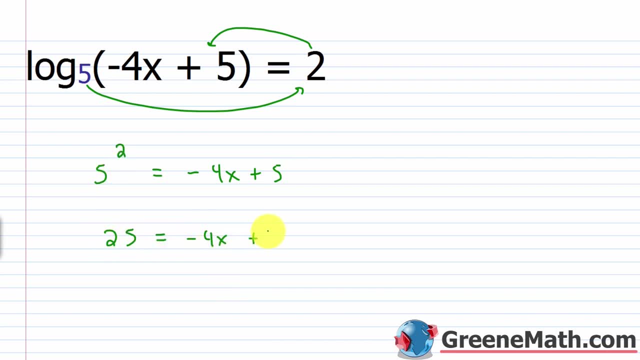 us 25.. This is equal to negative 4x, So we'd have 4x plus 5.. We will subtract 5 away from each side of the equation: 25 minus 5 is 20.. And this equals negative 4x. 5 minus 5 is 0. So divide both sides of the equation by negative. 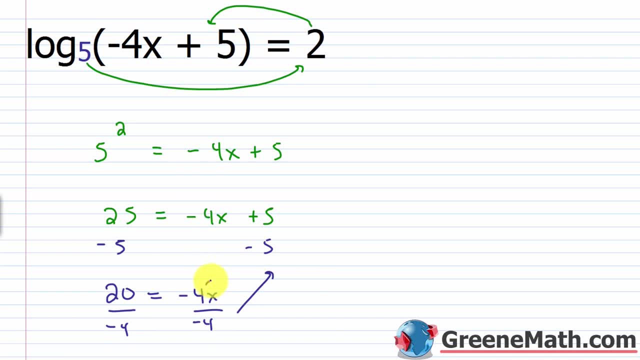 4.. This will lead us to this cancels. with this, We'll have 20 divided by negative 4, which is negative 5.. This is equal to x. So x equals negative 5.. Again, we can check this very. 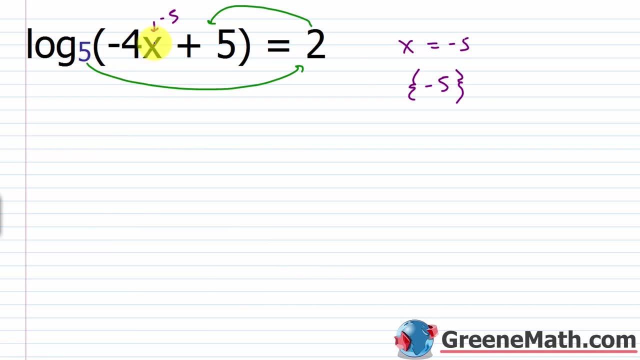 easily. So if I plugged in a negative 5 there- negative 4 times negative- 5 is 20.. 20 plus 5 is 25.. So in other words, is 5 squared equal to 25?? Yes, it is. So this guy right here checks itself. 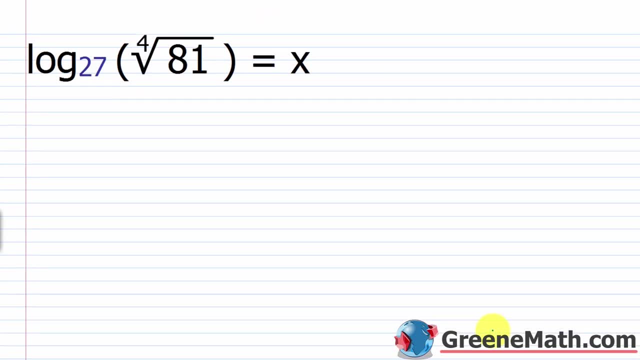 out All right. for the next one, we're looking at log base 27 of the fourth root of 81. This equals x, So we'd have 27 to. the power of x is equal to the fourth root of 81. we know is 3.. 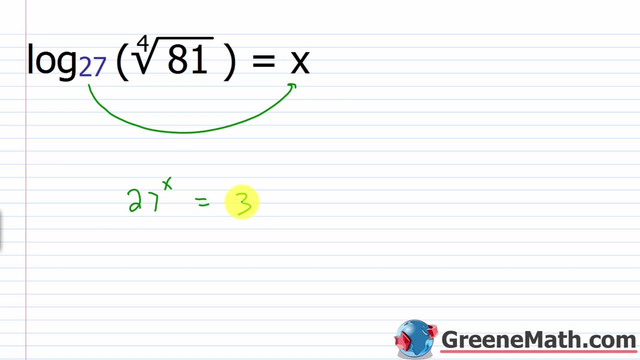 We have one where, again, if it's an exponential equation, we're thinking about solving based on having the same base and letting our exponents be equal to each other. So 27, we know, is 3 cubed. So I can use my power to power rule to kind of set this up. I can say this is 3 cubed. 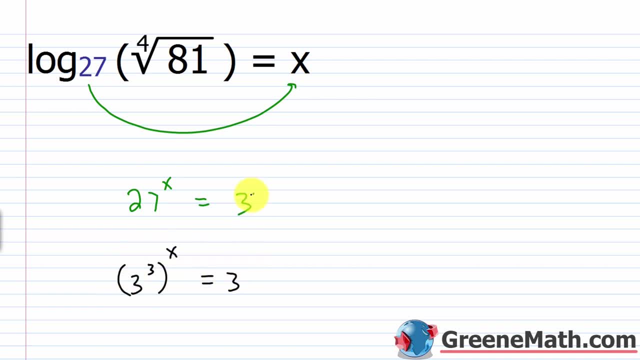 raised to the power of x equals 3.. And for the sake of this problem, we're going to write this as 3 to the power of 1.. All right, so we're going to write this as 3 to the power of 1.. 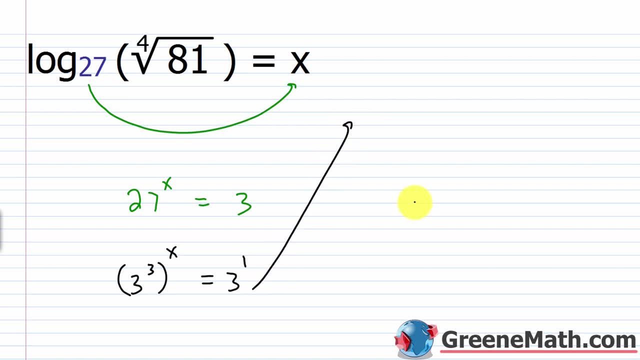 But then x1 is understood to be 1.. So transfer this guy up here. Power of power rule: if 3 is cubed and it's raised to the power of x, 3 stays the same. We multiply 3 times x to give us 3x. 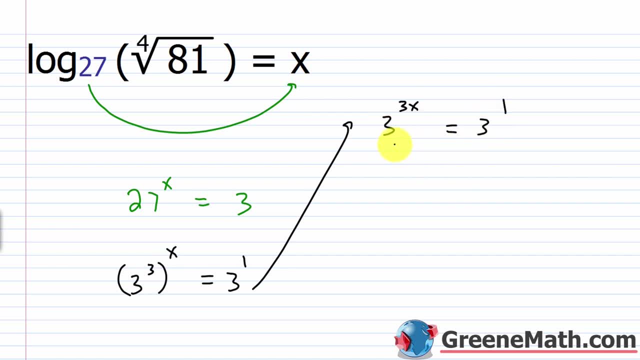 And this equals 3 to the first power. The base now is the same. So we have the same base. And we learned again in the last lesson: if the bases were the same you could set the exponents equal to each other. You could solve. So we would say 3x is equal to 1.. 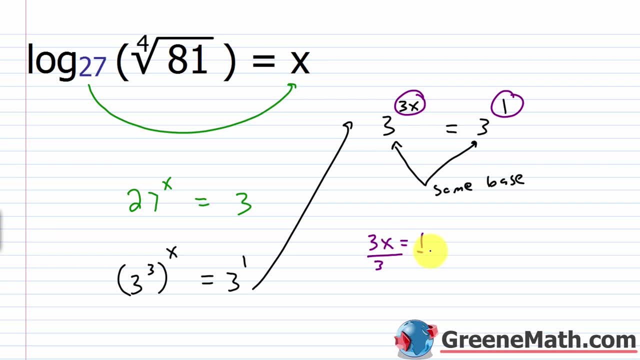 So 3x is equal to 1. Divide both sides of the equation by 3. You'll get x is equal to 1 third. So x equals 1 third. And again easy to check this. So if I plugged in a 1 third there, 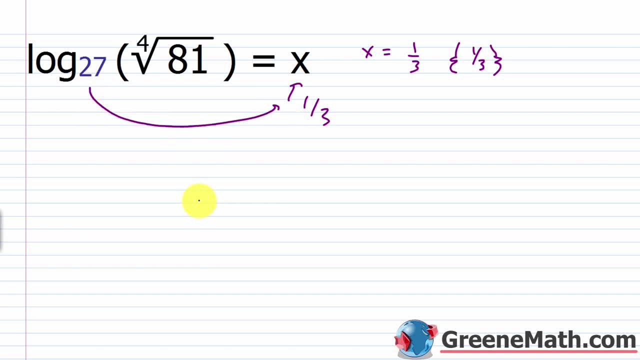 what would that tell me? Again, it's 27 to the power of 1 third would give me a result of the fourth root of 81.. The fourth root of 81 is 3.. So we know that's true. The cube root of 27,, which is: take something to the power of 1 third, you're taking the cube root. 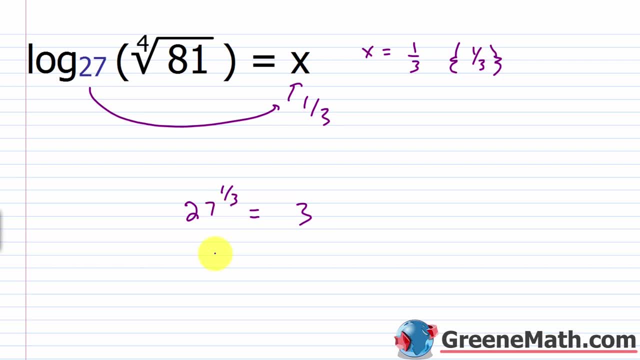 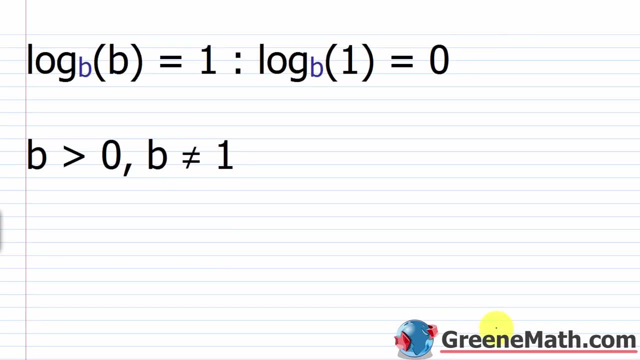 of it, The cube root of 27 is 3.. So you'd end up with 3 equals 3.. So this will check itself out as well. All right, let's think about some properties of logarithms. We'll learn about. 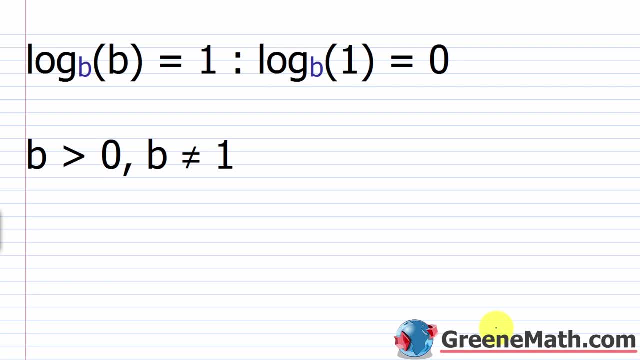 more properties of logarithms, ones that are a little bit more advanced in the next lesson, But for now let's look at these basic properties. So log base b of b is equal to 1.. This should make sense, because if you have some base, you're going to have some base. you're going to have some base. 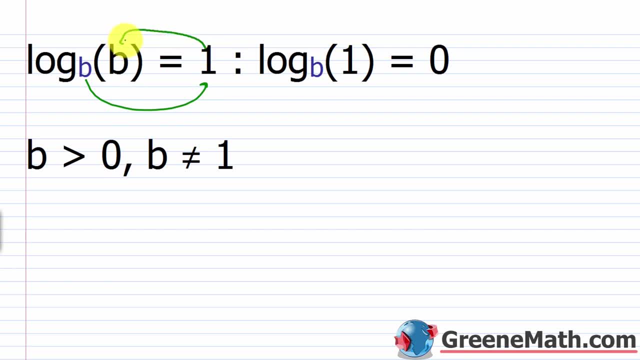 and you raise it to the power of 1, you would expect to get b back. Then log base b of 1 is equal to 0. So if I have a base b and I raise it to the power of 0, I should expect to get 1 back. 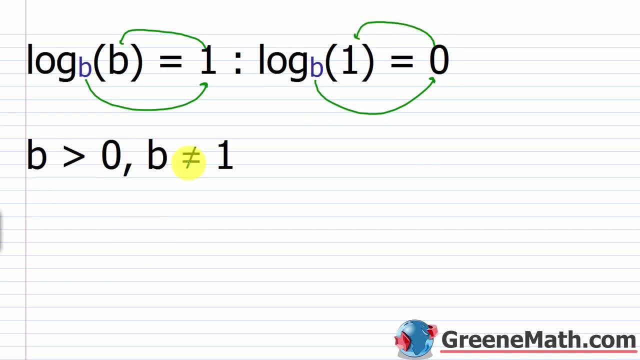 This is given the restrictions that b is greater than 0 and b does not equal 1.. So log base: 5 of 5 equals again very, very easy. 5 raised to what power would give me 5?? 5 raised to the first power. 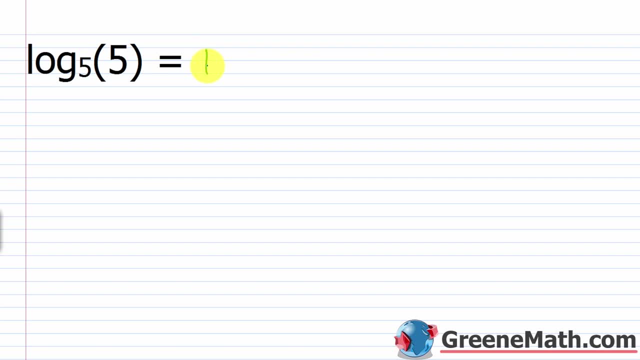 would give me 5.. And you could do a million examples of this. You could say: log base 1320 of 1320 equals what Again? this is 1.. Same number here and here Again, following those restrictions we gave, we know our answer is going to be 1.. All right, what about log base 105 of 1? Again. 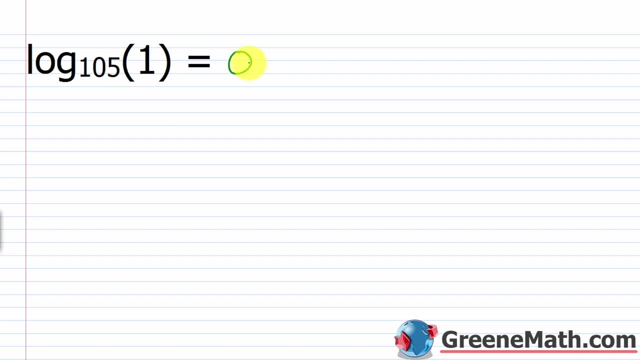 this is going to be 0, because 105 raised to the power of 0 would give me 1.. Again, another one to do. a million examples of, If I did like, log base 1 million of 1, again I know the result is 0.. 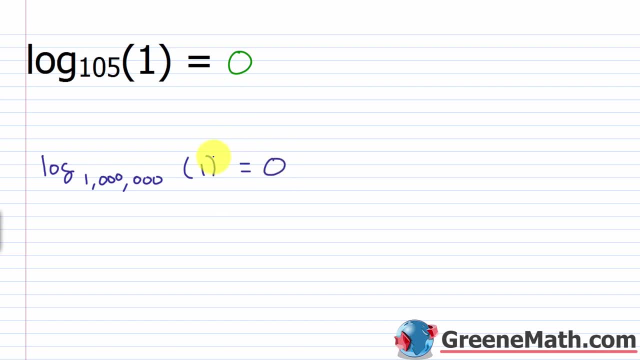 1 million raised to the power of 0 is 1, okay, If I did log base 20 million of 1, again I know the result would be 0.. Very, very easy if you come across those two scenarios. So let's kind of wrap. 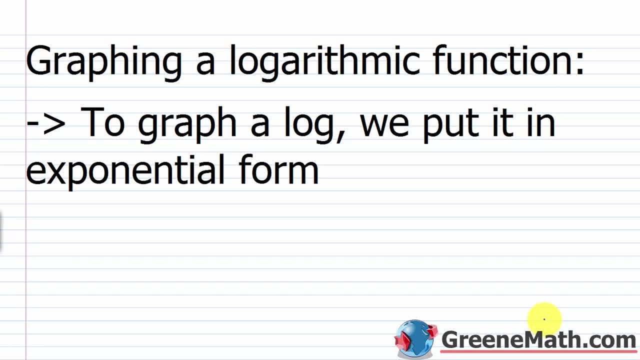 up the lesson by looking at some graphing. Now, at this point, we know how to convert between exponential form and logarithmic form, and we've seen how to solve some very basic logarithmic equations With graphing a logarithmic function. the first thing is to graph a log. 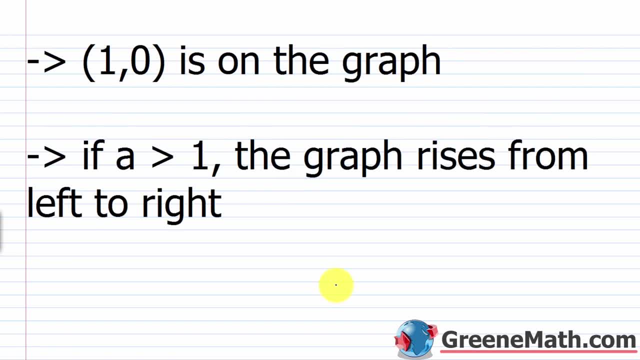 we put it in exponential form Now. remember that the exponential function and the logarithmic function are going to be inverses of each other. So when we looked at the exponential function, 0 comma 1 was always on the graph. Now, 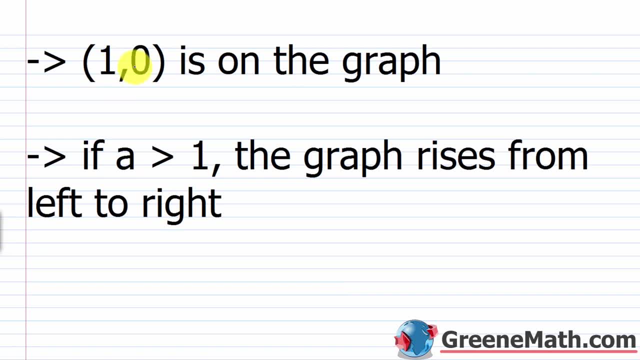 remember, the x and y's are interchanged with inverses, so 1 comma 0 is on the graph. So this was the y value from the exponential right when we talked about that. This was the x value from the exponential. So 1 swapped places right, It went from y to x. 0 swapped places, It went from. 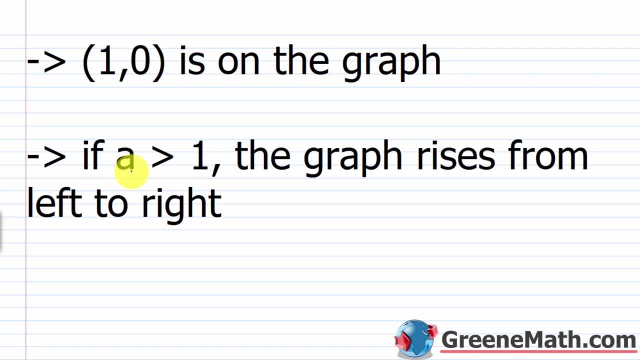 x to y. Now we say: if a is greater than 1, the graph rises from left to right. Then if a is greater than 0 and less than 1, it rises from left to right. So if a is greater than 1, it rises from. 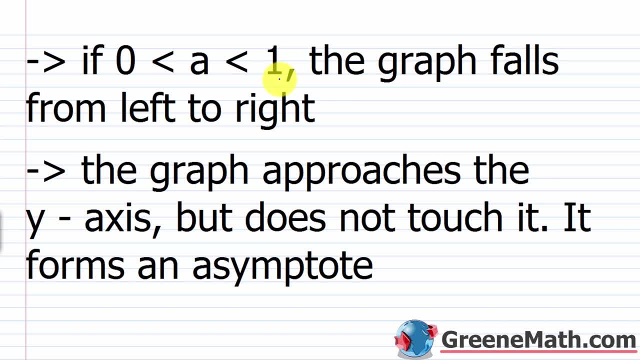 left to right. Now for this one. the graph approaches the y-axis but does not touch it. It forms an asymptote. So remember that we had an asymptote when we worked with exponential functions, but that guy was when it approached the x-axis. Think about what it means to approach. 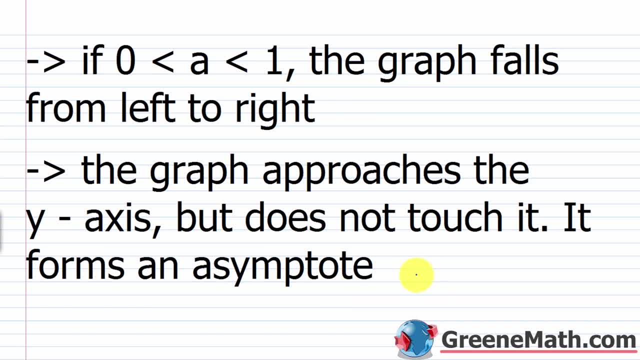 the y-axis. If you're looking at a coordinate plane, the y-axis is the value where x is 0. We said that if we had y equals log base a of x, that x was greater than 0. So we're telling you: 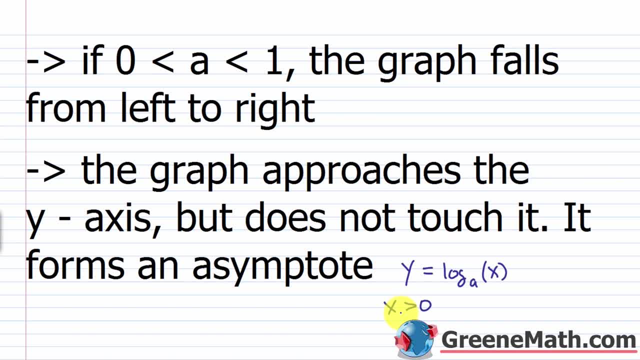 right there, hey, x will never be 0. So the graph will never actually touch the y-axis or a value where x would be 0. It's going to get infinitely close. The reason for this, again: if I have an exponential form, a to the power of y, that's going to be 0.. So if I have an exponential form, 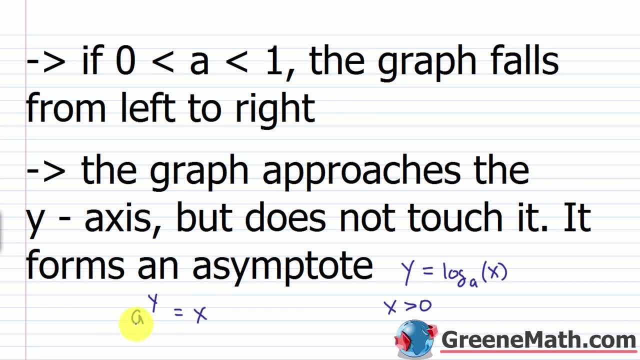 y is equal to x. Well, just think about this for a second Again: if a is restricted to be greater than 0 and a is not allowed to be 1, well then, when I take something positive here and I raise it to a positive value, OK, I'm going to get a positive result, I'm going to get something that's. 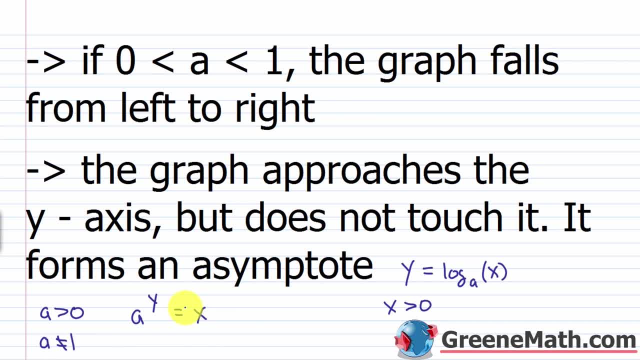 greater than 0. If I raise it to 0, I'm going to get 1.. If I raise it to something negative, I'm going to get a small number, but I'm never going to actually get to 0, right? So if I 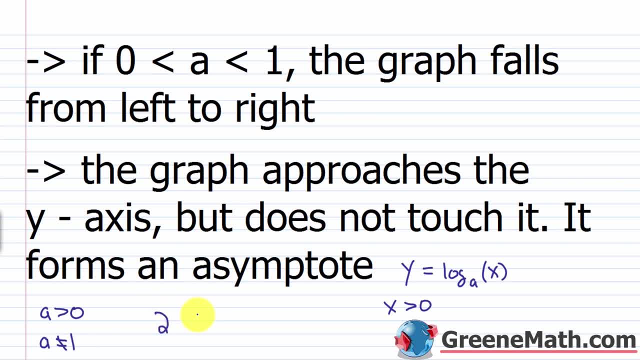 were to choose something like 2 to the power of I don't know some big negative, so let's say negative. let's say negative 10. This is equal to 1 over 2 to the 10th power That is going to be. 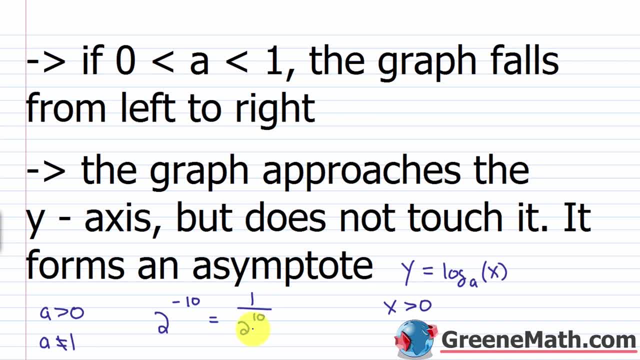 very close to 0.. And I can make this guy infinitely close to 0 by just making this part right here a bigger and bigger negative. Let's say I made this 2 to the power of negative 1 million. That's going to be really close to 0.. 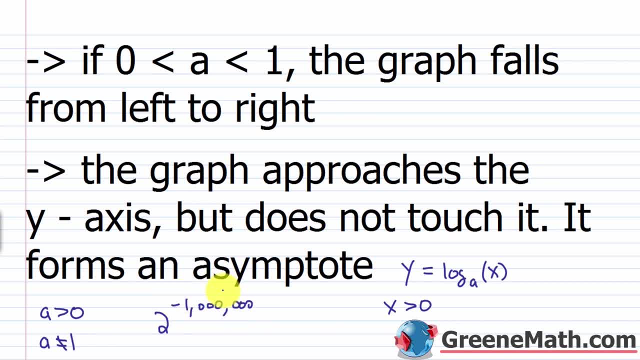 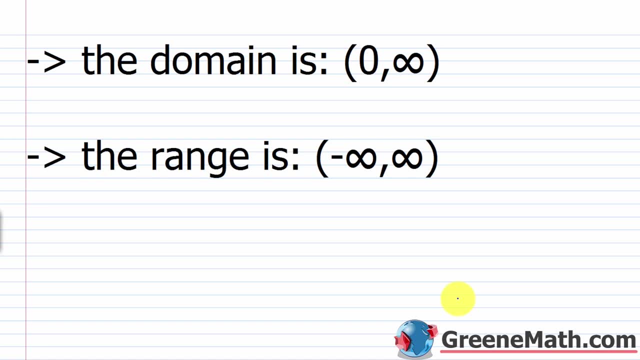 but I can keep getting closer and closer by just choosing bigger and bigger negatives right there. So it will approach the y-axis but it will never actually touch it. All right. so the domain and the range have flipped. The domain, when we looked at an exponential function, was all real numbers. 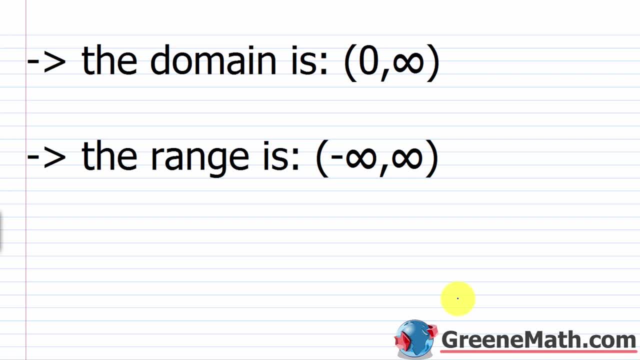 Now the domain is anything larger than zero. It can't be zero. we just talked about that. Anything larger than zero out to positive infinity. The range is anything from negative infinity to positive infinity, so it can be any real number. All right, so we're going to look at three graphs today. 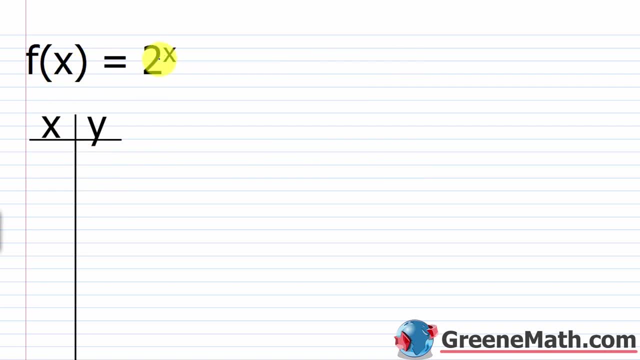 We're going to look at f of x equals 2 to the power of x. We're going to look at y equals x and we're going to look at the inverse of this guy right here, which is going to be a logarithmic function. 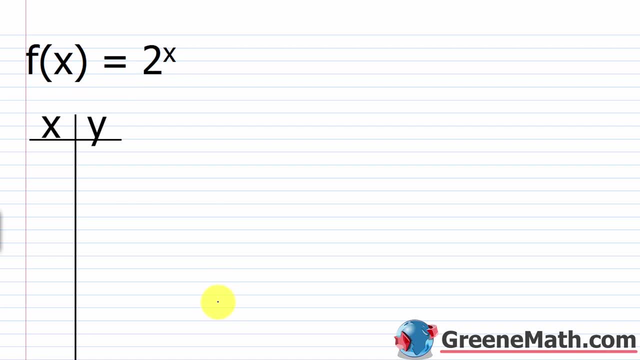 All right. so I'm going to start out by just getting some points here. So let's just choose some points like negative 3 for x, Let's do negative, 1 for x, Let's do 0.. Let's do 1, and let's do 3.. 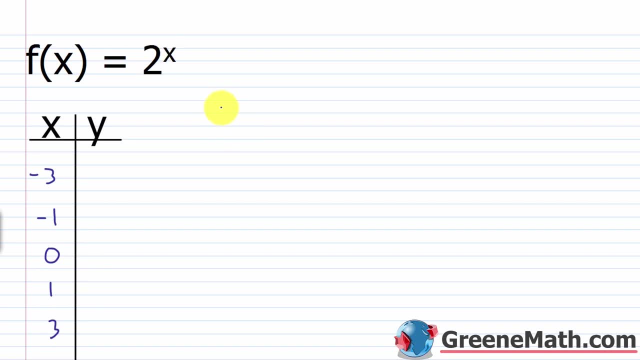 So if I plugged in a negative 3 for x, what would I get? We would have: y is equal to 2 to the power of negative 3.. This is 1 over 2 cubed, which is 1 over 8.. 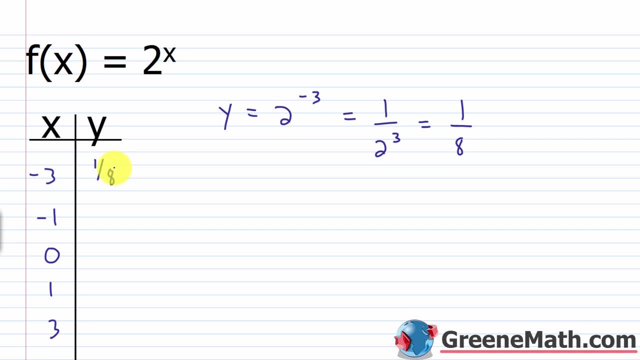 So if x is negative 3, y is 1. eighth, Then if x is negative 1, you can just think about plugging in a negative 1 there. This would be 1 over 2, which is 1 over 2.. 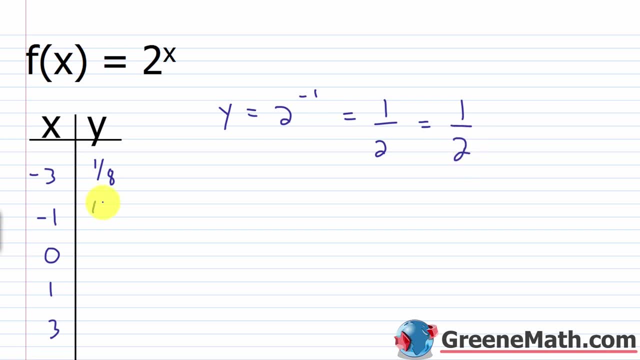 So we would have 1: half If x is 0, we know y is 1.. Right, 0 comma, 1 is always on an exponential function graph. And then if x is 1, y is going to be 2.. 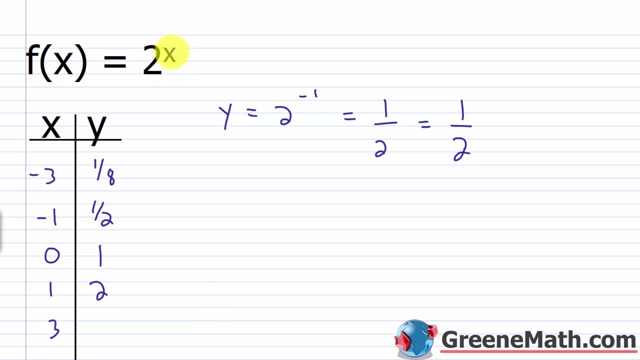 That one's very, very easy. If x is 3, right. if I plugged in a 3 there, 2 cubed would be 8.. So I've got 5 ordered pairs. So 5 ordered pairs. Let's go ahead and just plot those. 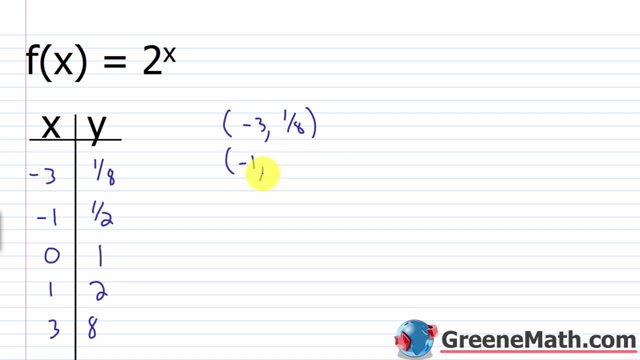 So we have negative 3 comma 1 eighth, We have negative 1 comma 1 eighth. We have negative 1 comma 1 half, We have 0 comma 1.. We have 1 comma 2.. And we have 3 comma 8.. 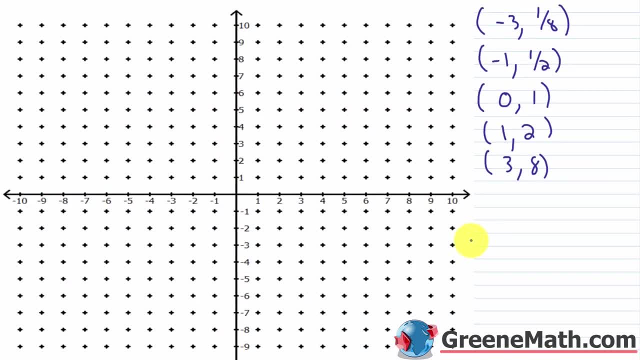 All right, we'll paste those guys. Let's just graph this guy real quick. So negative 3 comma 1 eighth. So negative 3 and then 1 eighth. We just got to kind of put a dot right there. We don't know exactly where it is because of our scale. 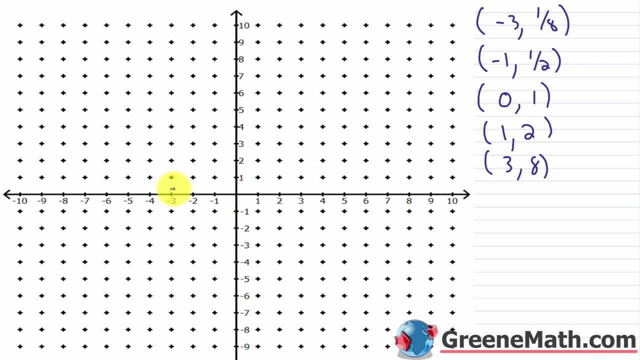 but let's just say that's pretty close. Then negative 1 comma 1 half. So we'll do negative 1 on the x-axis and then about halfway up here. So let's just say that's right there. 0 comma 1, that's easy. 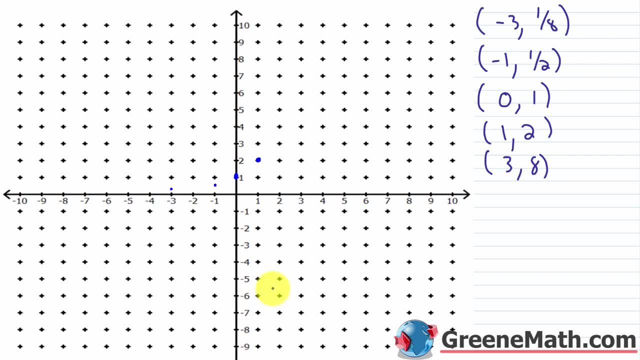 That's right there. 1 comma 2, another easy one, That's right there. And then 3 comma 8, that's easy as well, Okay. So again, as the x values get more and more negative, the graph approaches the x-axis. 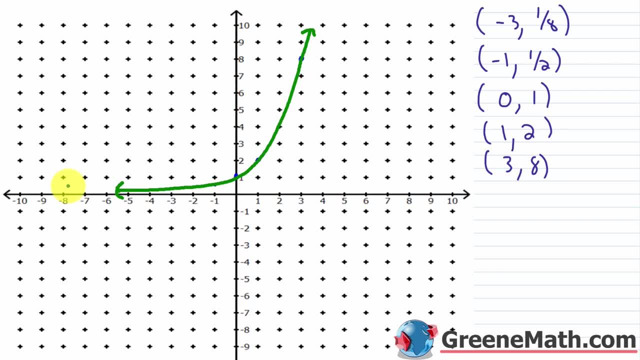 So it gets infinitely close to that guy, but it's never going to actually touch it. All right, so let me label this: This is the graph of f, of x is equal to 2 to the power of x. Now, the next one we want to graph is: y equals x. 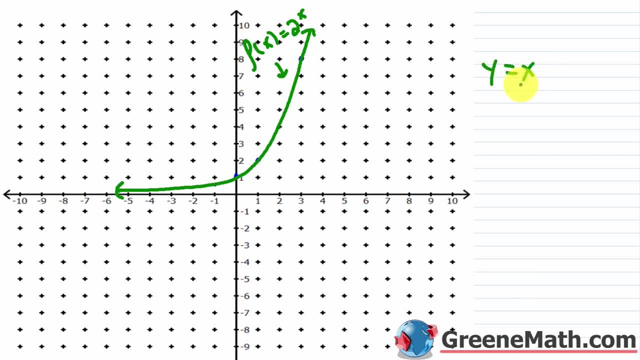 So if I graphed y equals x, I don't need to really get points going for that. So for this guy we know the slope is 1, right. Remember that y equals mx plus b, So a point on that line would be 0 comma 0, right. 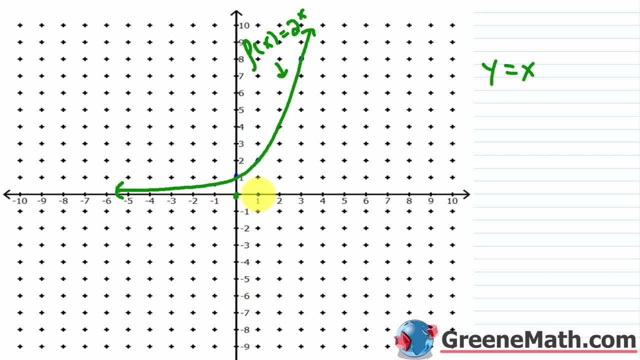 If x is 0, y is 0. So from there I can just use my slope of 1.. So to the right 1, up, 1.. To the right 1, up, 1.. To the right 1, up, 1.. 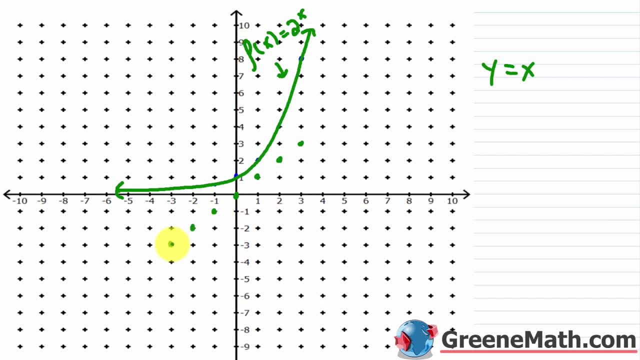 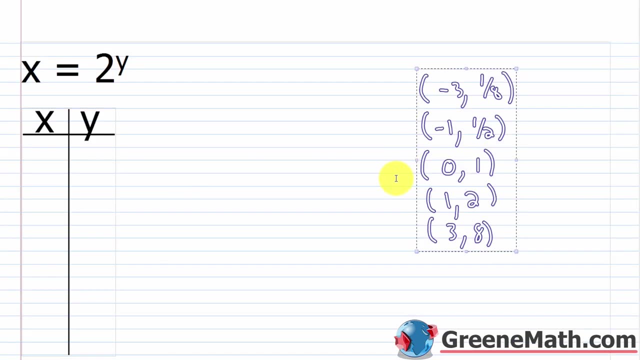 I could go down 1 to the left, 1, down 1 to the left 1, down 1 to the left 1.. Let me use a different color here, So we'll label this as f of x equals x. Okay, so let's go up to the last guy. 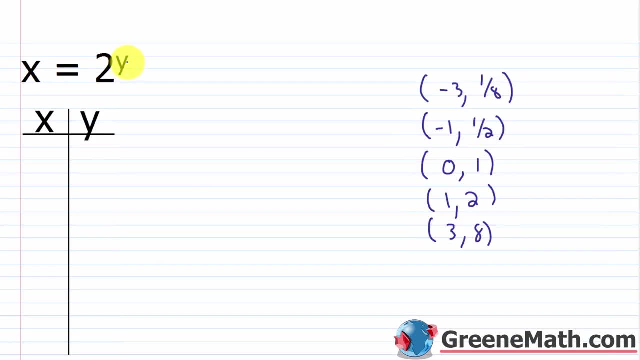 Okay, so we have x equals 2 to the power of y. Where did that come from? Again, if I have the inverse of f of x is equal to 2 to the power of x, I would first say f of x is y. 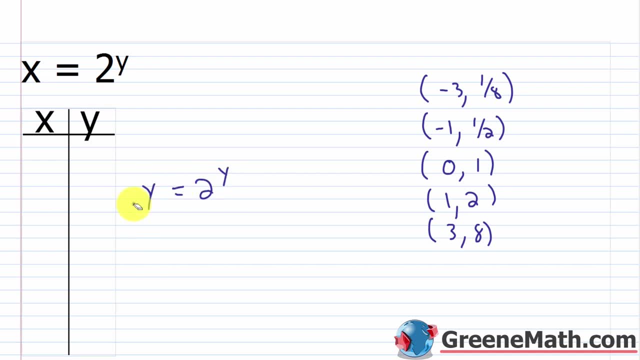 Then I would swap x and y, So this would be y and this would be x. Now I can write this in logarithmic form. I can say: y equals log base 2 of x, But again, when we're working with graphing, 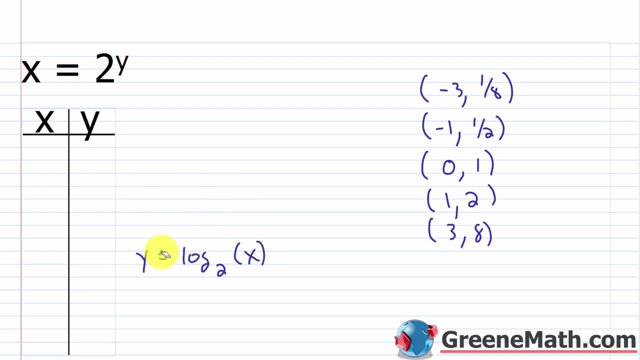 we want this in exponential form. So let's get rid of all this. Now you might say: why do you have these ordered pairs From the first guy we work with? When we work with, y equals 2 to the power of x. 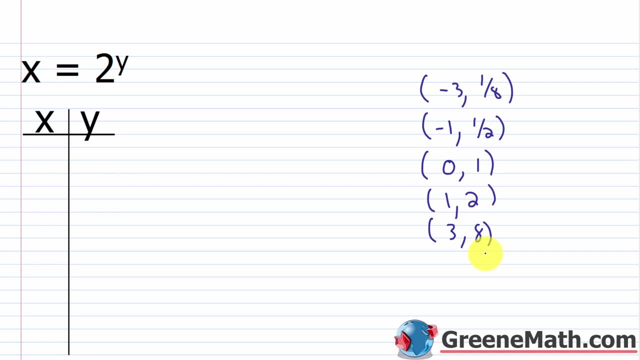 The reason is, if we have inverses, I can just flip the x and y values and I have ordered pairs. So, in other words, the x value of negative 3 would now be a y value of negative 3.. And a y value of 1 eighth would now be an x value of 1 eighth. 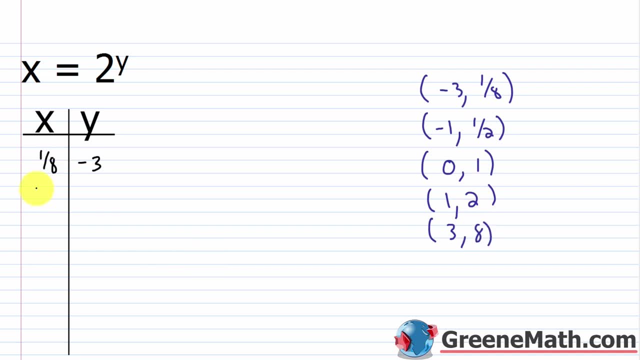 And I can just go down the list and just switch things. So, in other words, this would be 1 half, This would be negative 1.. This would be 1.. This would be 0.. This would be 2.. This would be 1.. 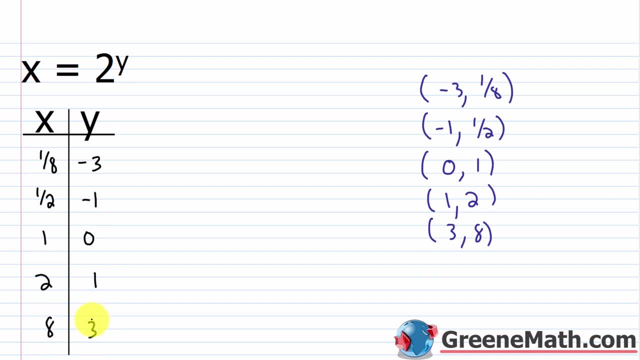 This would be 8.. This would be 3.. So you can check these if you want, but I can assure you that they do work. Let's just pick 2.. So if I took 2 and said this was equal to 2 to the power of 1,. 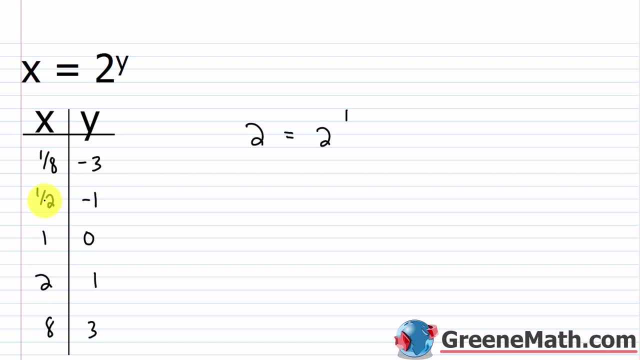 that checks itself out. You could take something like 1 half also. So 1 half is equal to 2 raised to the power of negative 1.. That's true, That would be 1 over 2 to the power of 1,. 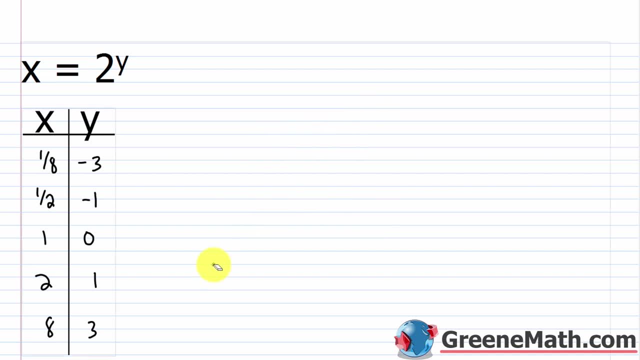 which is 1 half. All right, So now we can just set up our ordered pairs. So 1 eighth comma negative 3.. We have 1 half comma negative 1.. We have 1 comma 0.. We have 2 comma 1.. 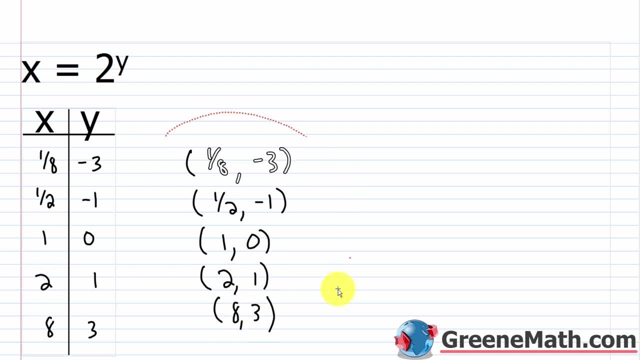 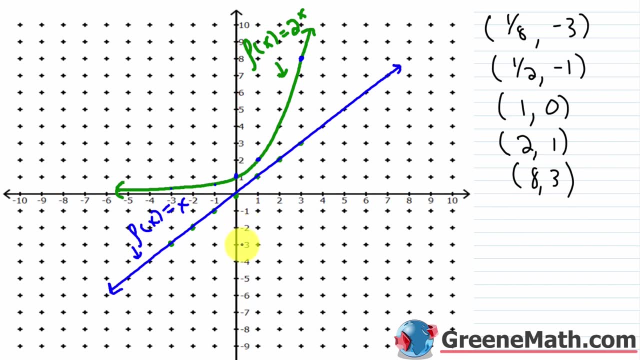 And we have 8 comma 3.. So let's copy these. So 1 eighth comma, negative 3.. So on the x-axis, 1 eighth is, let's say, about right there, Negative 3, we drop down 3 units. 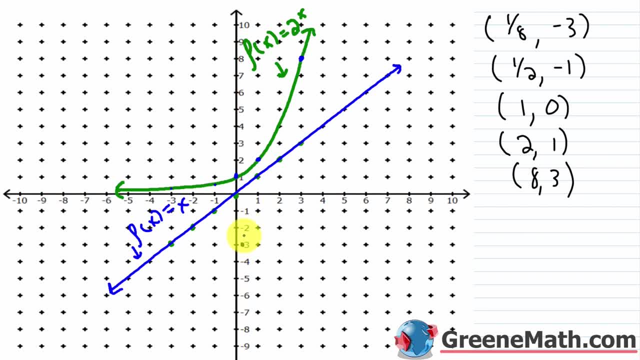 So let's just say the point's right there: 1 half comma negative 1.. So 1 half would be about right there. Negative 1 would be about right there: 1 comma 0. So that's right there. Then we have 2 comma 1.. 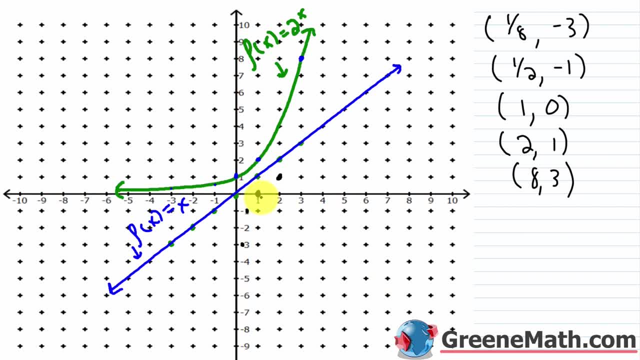 So 2 comma 1 is right there, And then 8 comma 3.. So 8 and then 3.. So remember, for this one, we're never going to actually be able to touch the y-axis As the y-values get more and more negative. 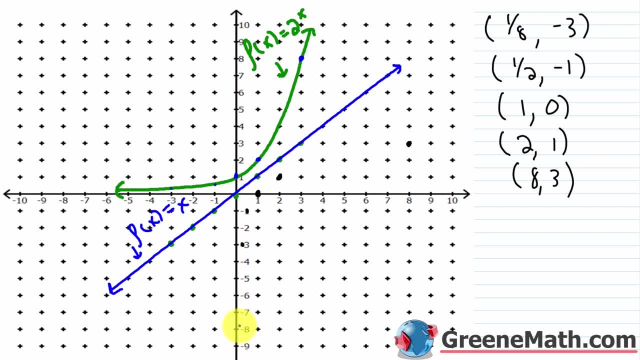 we're going to get closer and closer to the y-axis, or an x-value that is 0. But we'll never actually be able to touch it. Remember, x is strictly greater than 0. So So this guy right here is f of x, or y is equal to log base 2 of x. 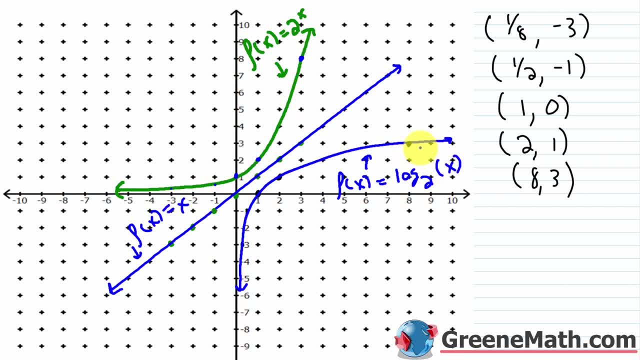 So, looking at the graph, we can see that we do have inverses. And again, the way you can kind of show this to yourself: if you've drawn that line f of x equals x or y equals x, and you do this at home, 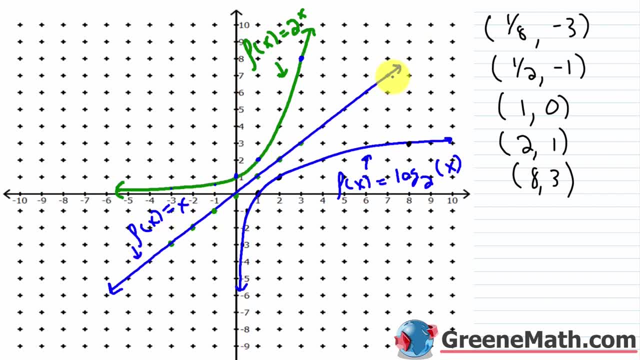 you can take your sheet of paper and you can fold the paper exactly on that line f of x equals x, And what's going to happen is this graph right here will be exactly on top of this graph right here, And that's how you can prove that you have inverses. 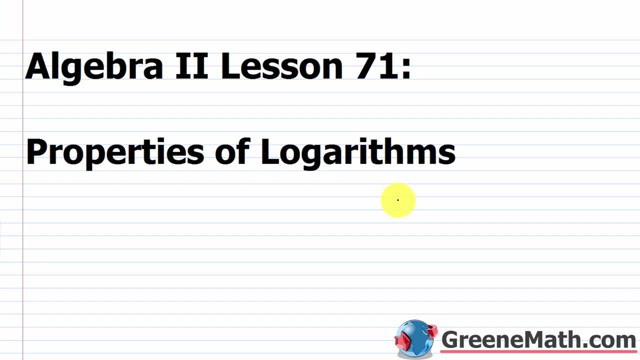 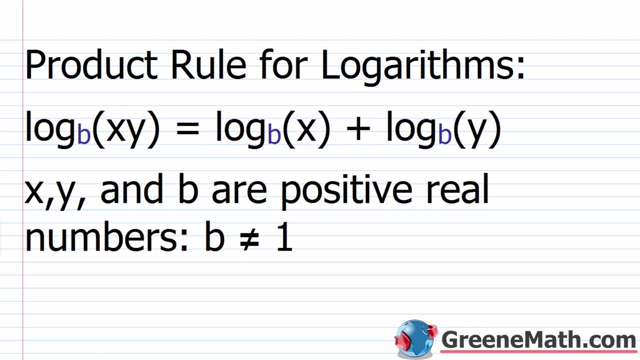 Hello and welcome to Algebra 2, Lesson 71. In this lesson we're going to learn about properties of logarithms. So in the last lesson we started talking about logarithms. We showed what a logarithm was And we showed how to go back and forth between exponential form. 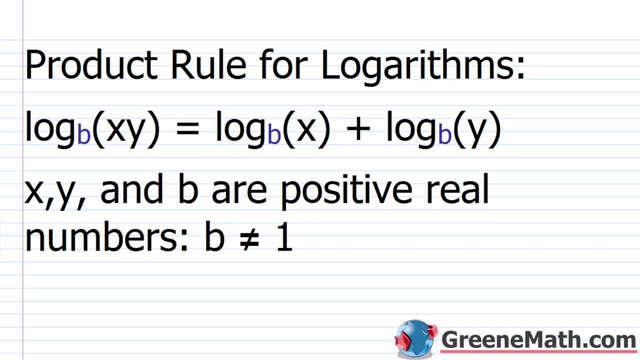 and logarithmic form. Now, in this lesson, we're going to dig a little bit deeper. We're going to talk about some of the properties that you're going to encounter when you're studying logarithms. So the first property you're likely to come across- 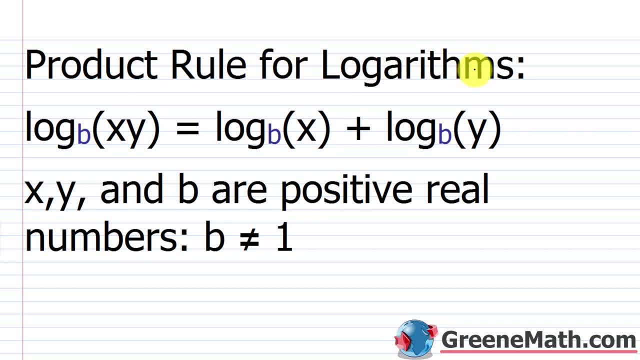 is known as the product rule for logarithms. So if you see something like log base b of xy, this is equal to log base b of x plus log base b of y. So what is this telling us? Well, essentially what it's doing. 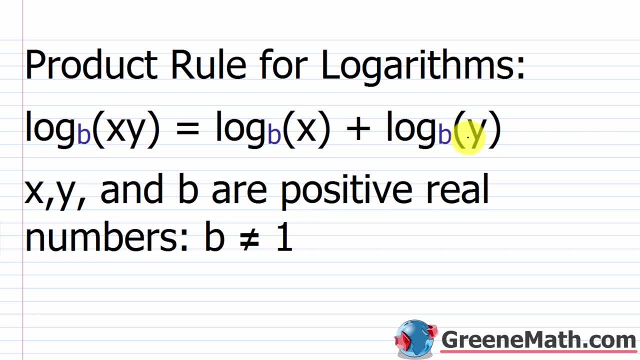 is. it's allowing us to write multiplication as addition. So in your book you'll probably read: the logarithm of a product is the sum of the logarithms of the factors. So let's reflect on that for a minute. I start out with log base b of x times y. 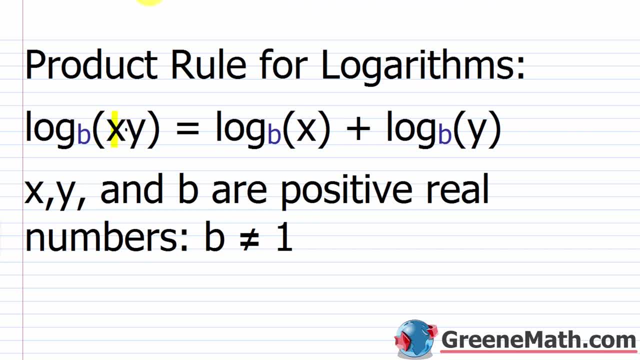 So we can think of x as a factor and we think of y as a factor. right, Those two are being multiplied together And we expand this into. we say: this is equal to log base b, so the base is the same of x. x is the first factor. 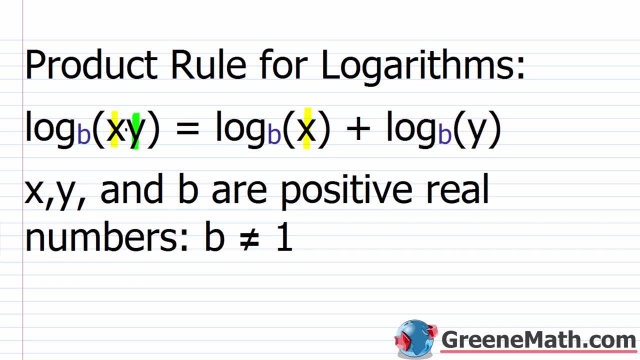 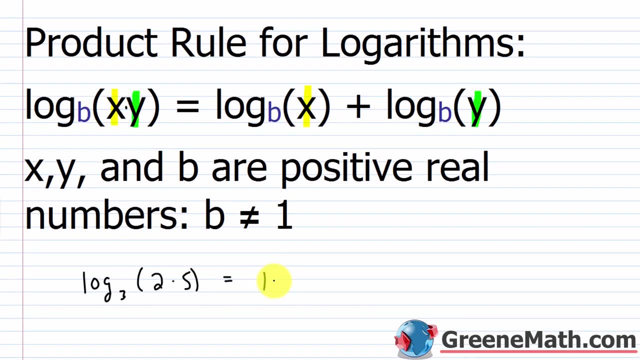 then plus log base b of y. y is the second factor. So if I saw something like log base 3 of I don't know, let's say 2 times 5, this would be equal to log base 3 of 2. 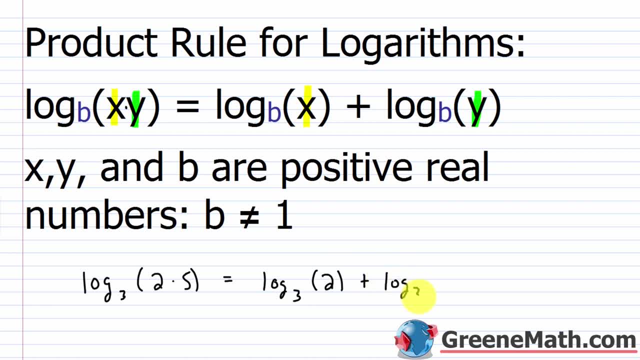 plus log base 3 of 5.. Okay, very, very simple. You just take your first factor and put it there. your second factor goes there. Very, very easy to do this. Now there are some restrictions. We say x, y and b. 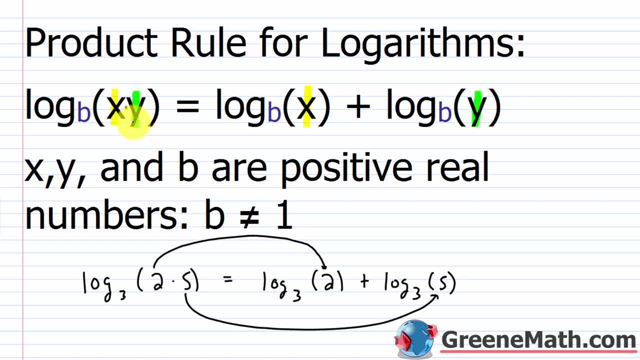 So x and y are the factors here, and it could be more than x and y. You could have three factors, four, you could have as many factors as you want, But all those factors have to be positive real numbers, so greater than zero. 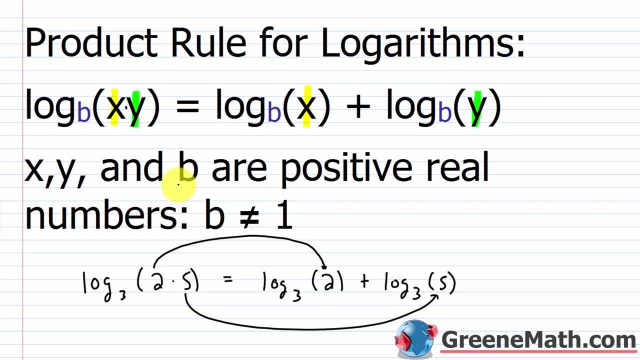 Now b: the base has to be a positive real number, and then, in addition to that, we have this added restriction: b has to be not equal to the number 1.. So it has to be a positive real number and it can't be 1.. 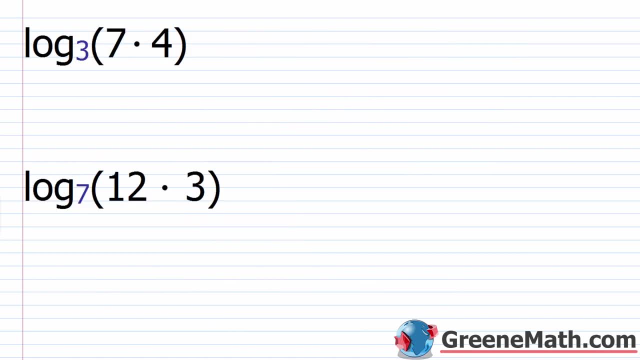 All right. so let's take a look at a few easy examples here. If we saw something like log base 3 of 7 times 4, again, all I'm going to do is just expand this. So this tells me I could rewrite this as log base 3 of 7,. 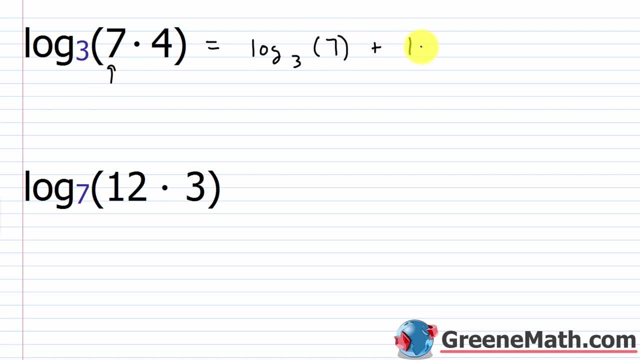 right, my first factor, plus log base 3 of 4,. right, my second factor. So this guy went here and this guy went there. Very, very easy. okay, Same thing here. So log base 7 of 12 times 3,. 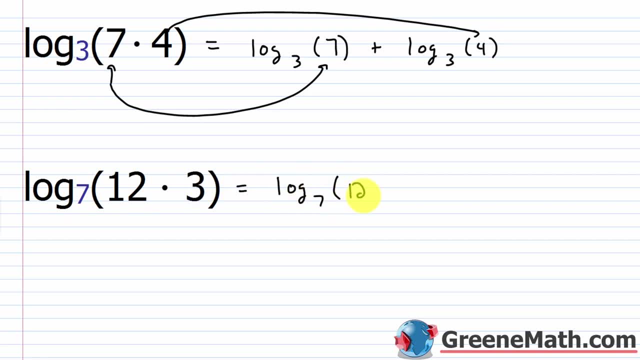 this is log base 7 of 12, then plus you have log base 7 of 3.. All right, Let's take a look at another one. So we have log base 2 of 5 times 12.. So it's log base 2 of 5 plus log base 2 of 12.. 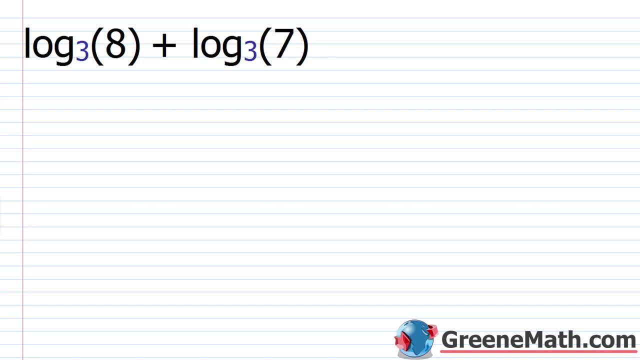 Very, very simple. All right, now let's try to reverse the process. You might be asked on your homework or on a test to condense, So using the same property that we just talked about. if I saw log base 3 of 8,. 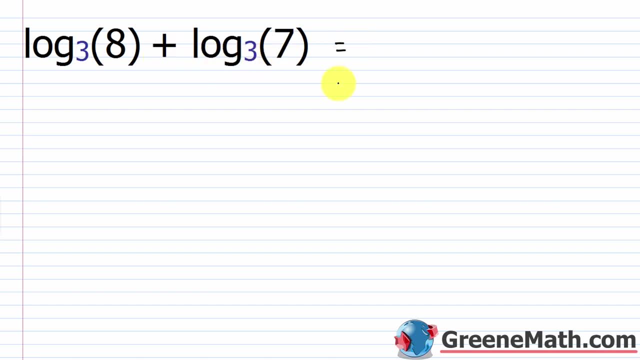 plus log base 3 of 7, I know I could rewrite that as log base 3, right log base 3 and log base 3, so it's just going to be log base 3 of. you've got an 8 here and a 7 here. 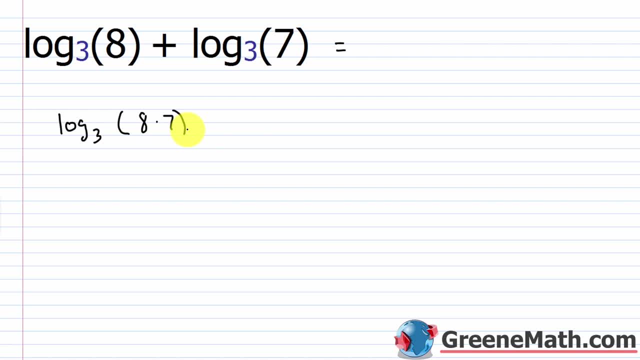 So you would have 8 times 7, or you could really multiply those two together and say it's 56, if you wanted to. So let's say this is equal to log base 3 of 56.. What if you saw log base 4 of 11?? 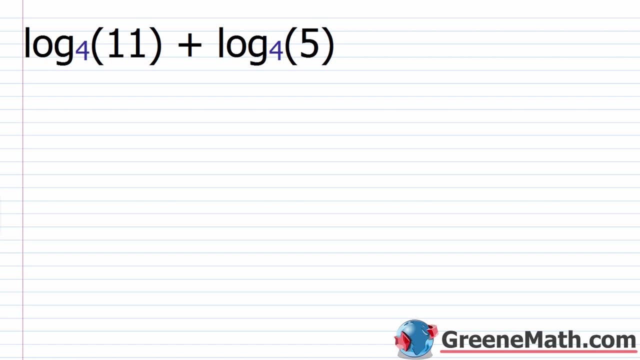 Plus log base 4 of 5.. So log base 4, log base 4.. So it's going to be log base 4.. And then of you have 11 here and 5 here, So those are going to be multiplied together. 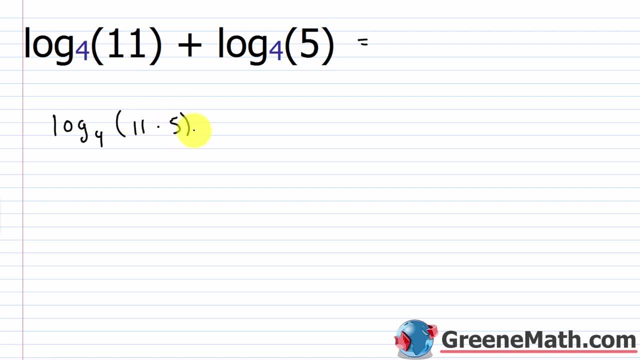 So it would be 11 times 5,, which we know is 55, so we could write it as log base 4 of 55.. Let's take a look at another one. So if you saw something like log base 8 of 7,. 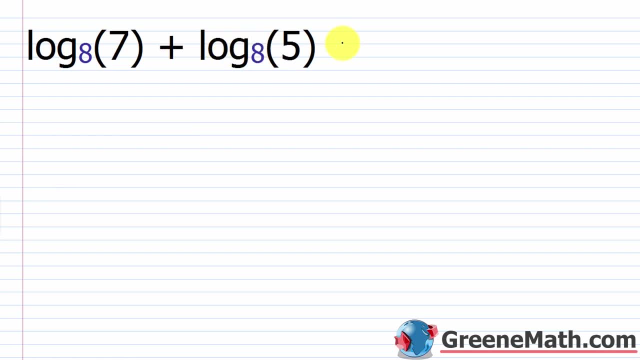 plus log base 8 of 5, what would you do? You have that log base 8, so that's log base 8 of. you've got a 7 here and a 5 here. So 7 times 5 would give me 35.. 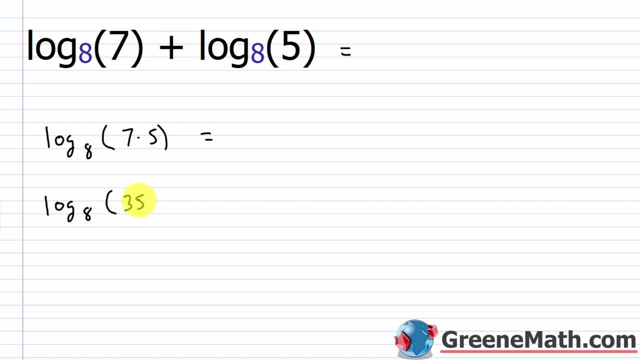 So log base 8 of 35.. Alright, so very, very easy to deal with the product rule for logarithms. The quotient rule for logarithms is just as simple, So let's take a look at that. So if we see log base b of x over y, 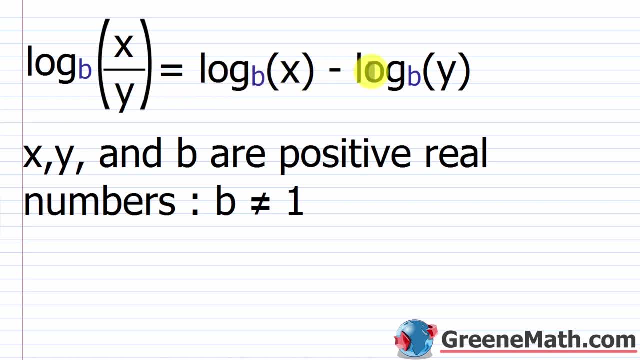 this is equal to log base b of x minus log base b of y. So, in other words, the x in the numerator is going right here, The y in the denominator is going right here. So this is subtraction, whereas when we talked about the product rule, 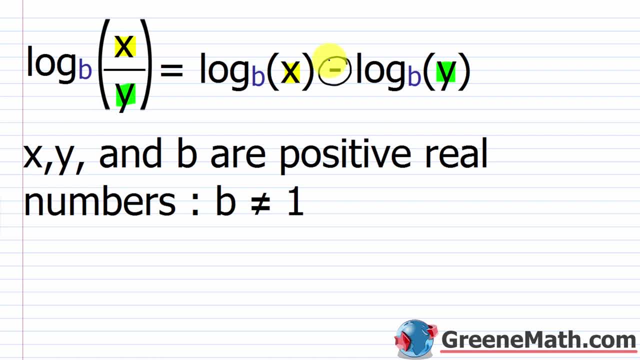 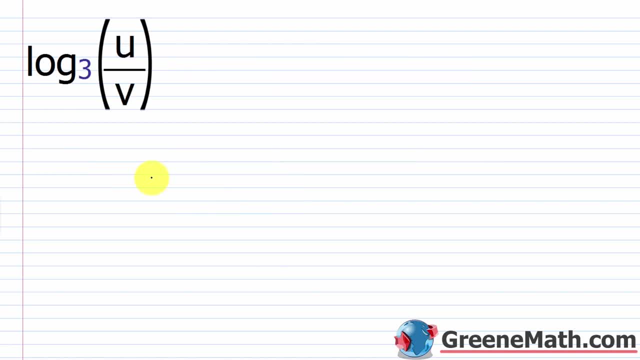 it was addition. Okay, it was addition. So we have the same restrictions. x, y and b are positive real numbers And b is not allowed to be equal to 1.. Alright, for the first one. we have log base 3 of u over v. 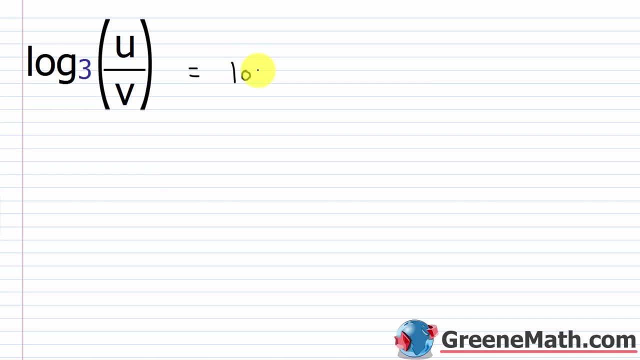 So, in other words, what I'm going to do is I'm going to say we have log base 3 of what's in the numerator, That's a u, Then minus. we'll have log base 3 of what's in the denominator. 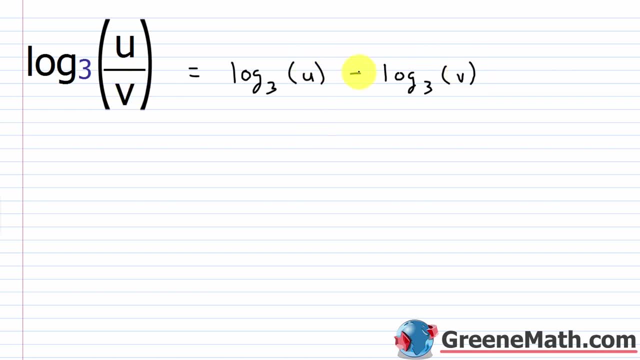 That's v. It's always numerator here. You'll have your minus sign denominator here. Okay, the log base 3 will be the same in each case. So you've just got to work out what's going to go in this position and what's going to go in this position. 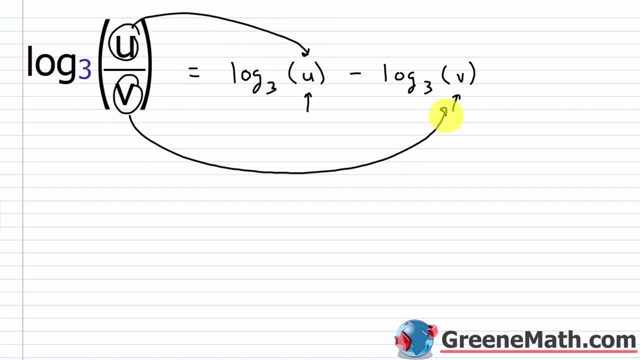 Again. numerator is going to go here. Denominator is going to go here. Alright, for the next one, we have log base 8 of 12 over 11.. So this is going to be log base 8 of 12,. 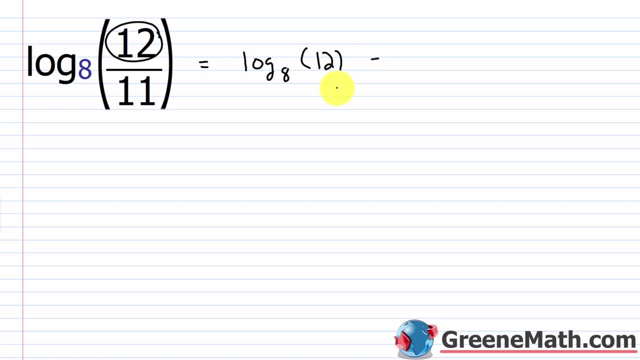 what's in the numerator minus? you'll have log base 8 of 11.. What's in the denominator Alright, now we have log base 5 of 3 over 7.. So this is going to be equal to log base 5 of 3. 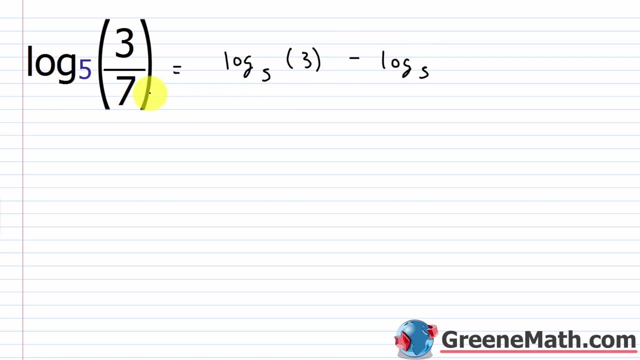 minus log base 5 of 7.. Alright, so now let's talk about reversing this process. So if I saw something like log base 9 of 10 minus log base 9 of 7, what would I do? Well, I know that I would have log. 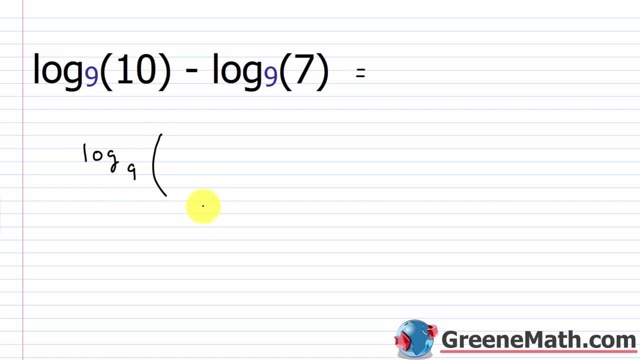 base, not Then of what. Well, I know it's this guy. The first one that appears is 10.. That's going to go in my numerator, And then it's over. The second guy that appears is 7.. That's going to go in my denominator. 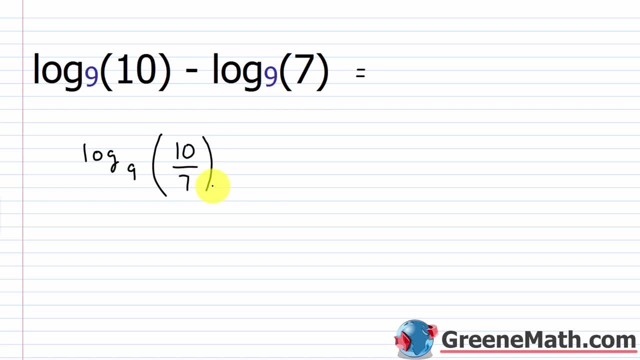 So this becomes log base 9 of 10 over 7.. Alright, for the next one. we have log base 10 of 7 minus log base 10 of 11.. So we know this is going to be log base 10 of. 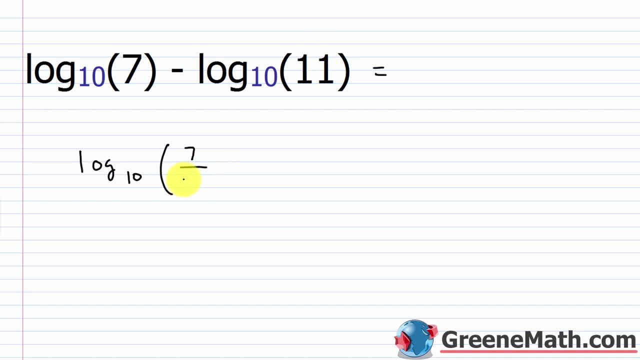 you'll have 7, over, then you'll have 11.. You just want to go in order. So 7 is first, so it goes in the numerator. 11 is second, so it goes in the denominator. So again, log base 10 of 7 over 11.. 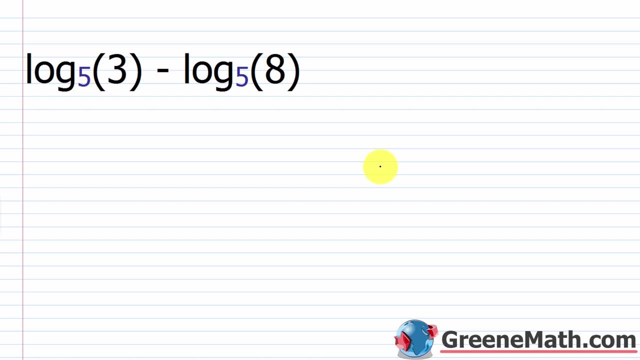 Alright, for the next one. let's look at log base 5 of 3 minus log base 5 of 8.. So, again, very, very easy. This is going to be log base 5 of the one that appears first is 3,. 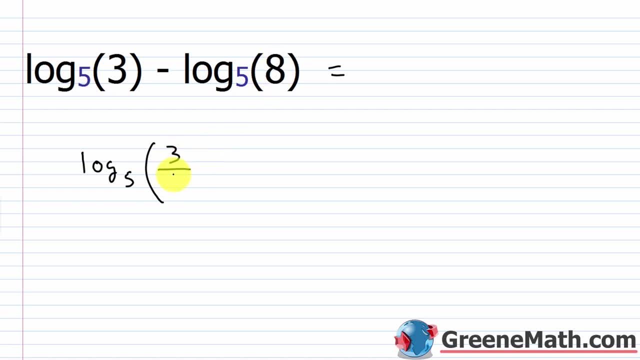 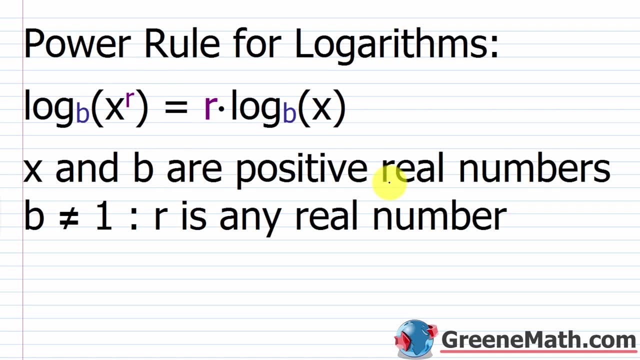 so that goes in my numerator over the one that appears. second is 8, so that goes in my denominator. So this is log base 5 of 3 over 8.. Alright, so now we have the power rule for logarithms. 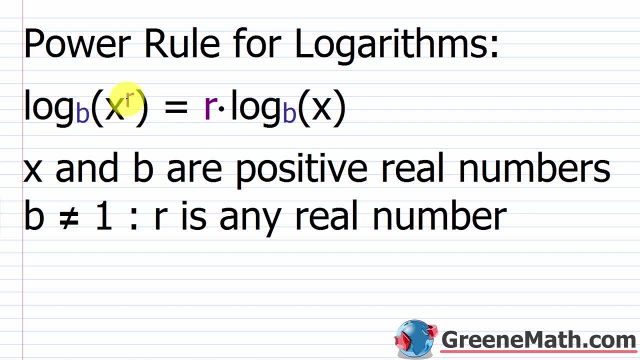 So you have log base b of x to the power of r. We say this is equal to r, which was the exponent here, multiplied by log base b of x. So in other words, the exponent just comes down and goes in front. 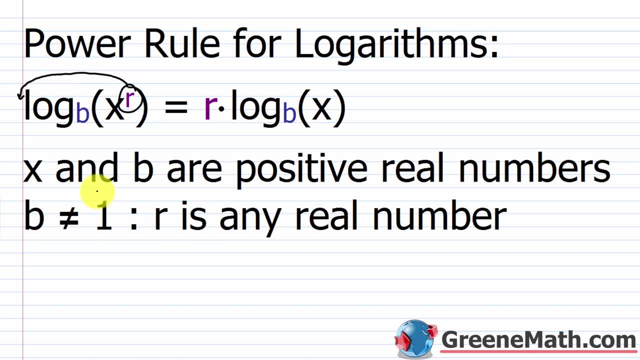 Okay, that's all we're doing there. So again, x and b are positive real numbers and b, again, is not allowed to be equal to 1 or is any real number that you'd like. So it can be negative, it can be positive. 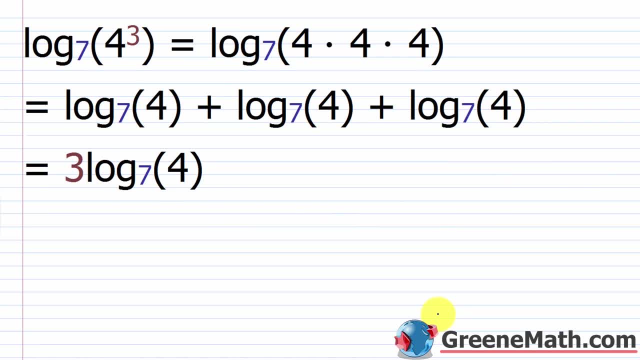 it can be 0,, whatever you'd like it to be. So to give you kind of a quick example of why this occurs, let's say you saw log base 7 of 4 cubed. We could write this as log base 7 of 4 times 4 times 4.. 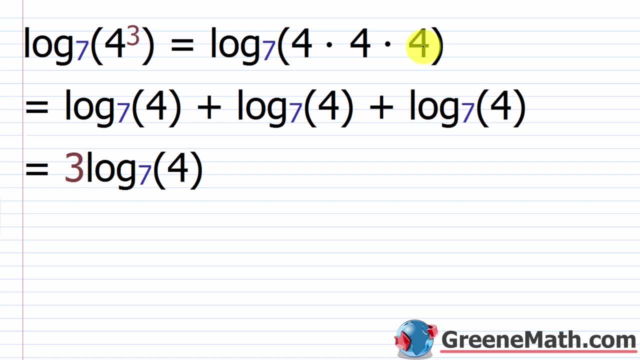 Now, using our product rule that we learned earlier, we could expand this and say: this is log base 7 of 4 plus log base 7 of 4 plus log base 7 of 4.. So I have 3 of the same thing. 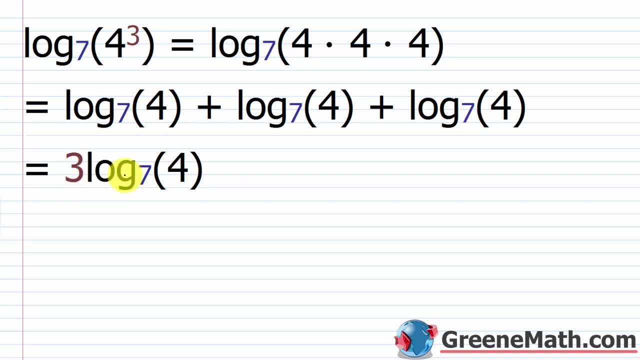 So I can just say I have 3 times that thing, which is log base 7 of 4.. So that's all we're doing here. We're not doing any magic tricks. So if I saw log again, base 7 of 4 cubed. 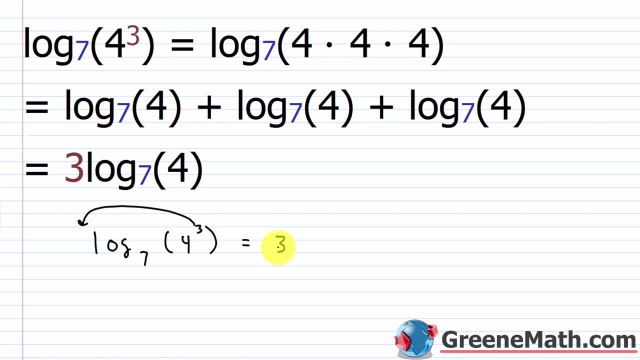 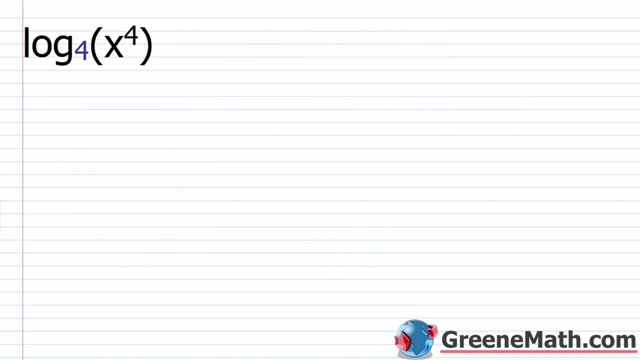 this guy just goes in front. So we just say this is 3 times log base 7 of 4.. Very, very easy, All right. so what about log base 4 of x to the fourth power? Again, this guy is just going to go out in front. 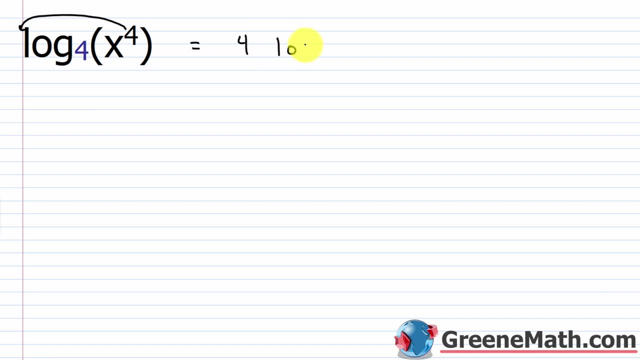 So this is equal to 4 times log base 4 of x. What about log base 5 of the square root of x? So for this guy, you want to write it where you have a fractional exponent. So you're going to say this is log base 5. 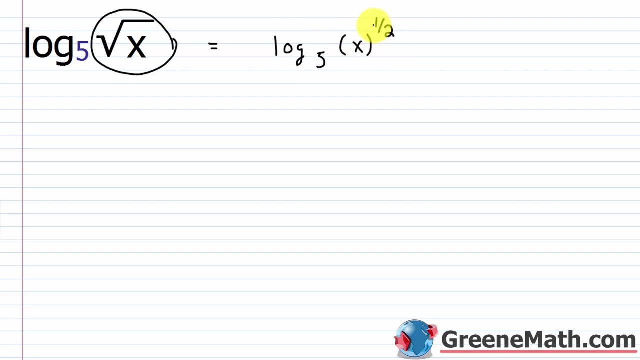 of x raised to the power of 1 half, And then you just want to bring this guy down. So this is going to be equal to 1 half multiplied by log base 5 of x. What about log base 8 of the cube root of x? 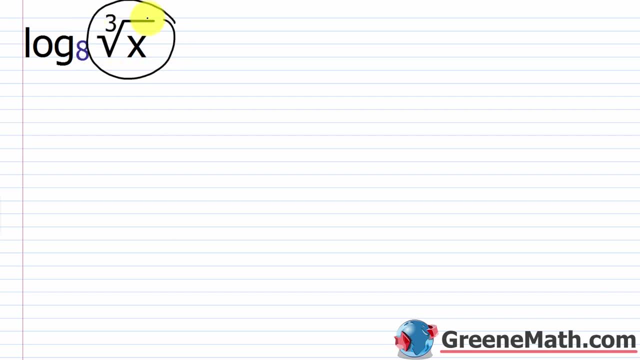 Again. you want to write this using a fractional exponent, So you would say this is log base 8 of x raised to the power of 1 third. This will be equal to again bring this guy down. So this will be 1 third times log base 8 of x. 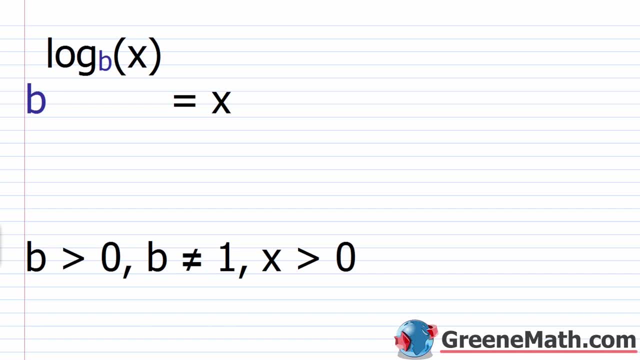 All right, now let's talk about two special properties that you're going to come across in this section, And when you first look at them, they might look like gibberish, but they really save you a lot of time if you can identify them when you're doing your homework. 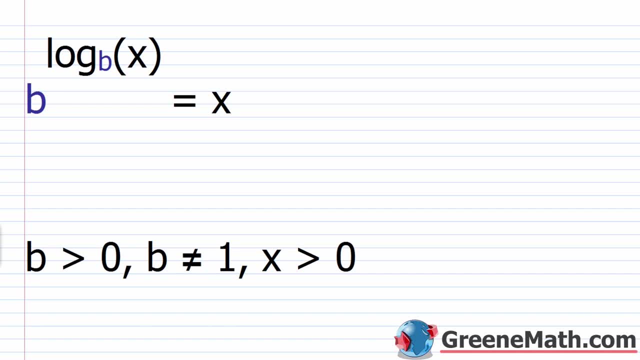 or if you're on a test or really any practice that you're doing. So if you see something like b raised to the power of log base b of x, you should know this is equal to x. Now, the restrictions here is that b has to be greater than 0,. 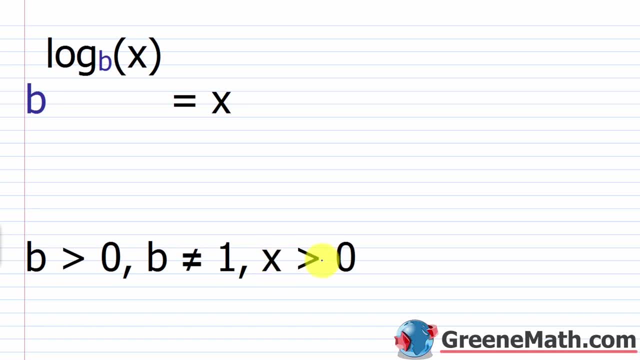 b is not allowed to be equal to 1, and x is greater than 0. So as long as those criteria are met, we're going to be good to go with this kind of formula here. And just to demonstrate this, I think when you see a numerical example. 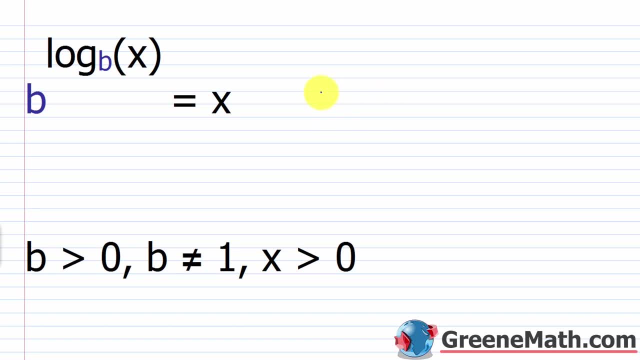 it'll make more sense for you If you see something like 3 raised to the power of log base 3 of 7, what would this be equal to? Well, from just looking at this, from just looking at this over here, 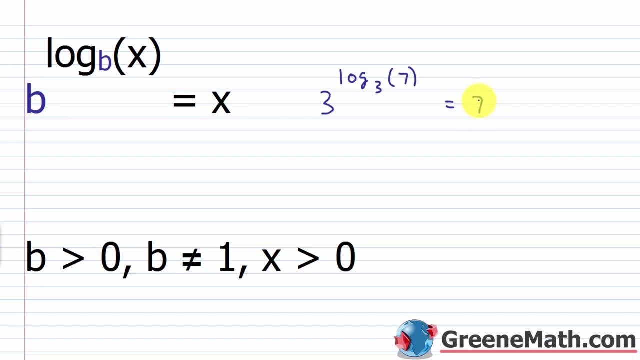 you can kind of compare things and say: well, I know it would be equal to 7, because this guy right here, this b is here and here I have a 3 that's here and here, right. So 3 is kind of in the place where b is in the generic formula. 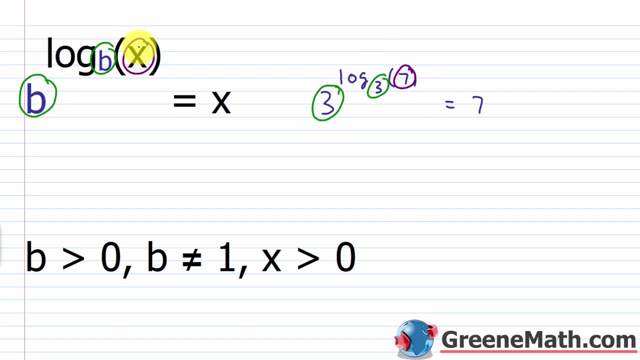 Then if I know that 7 is here where this x is here, and then there's an x here, so a 7 must go there. So by that process you can kind of figure it out. But you really want to understand where we get the answer of 7.. 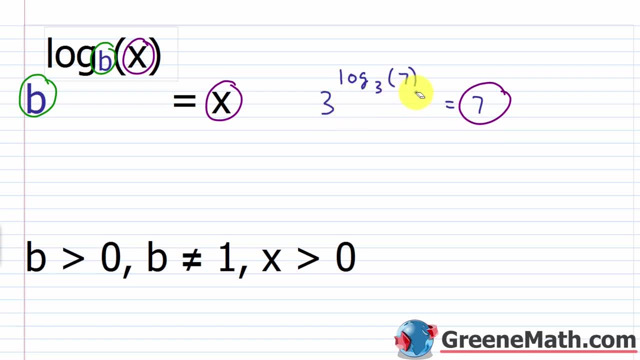 It's a lot easier than just kind of looking at things and saying, oh, the generic formula says this, so let me just copy that. Think about what this part is right here, independent of anything else, If I have a log base- 3 of 7,. 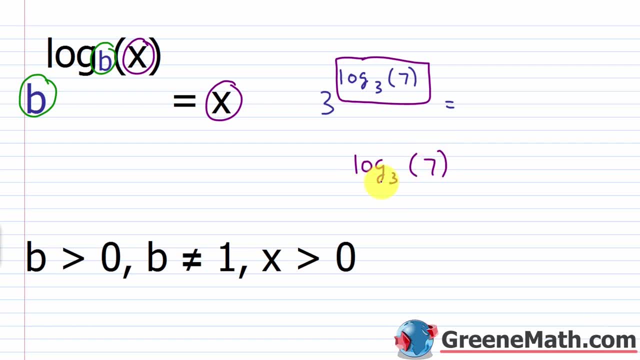 this is the exponent that 3 must be raised to to obtain 7.. Well, my base here is 3.. This is a base of 3.. 3 is basically. 3 is being raised to this guy right here, which again. 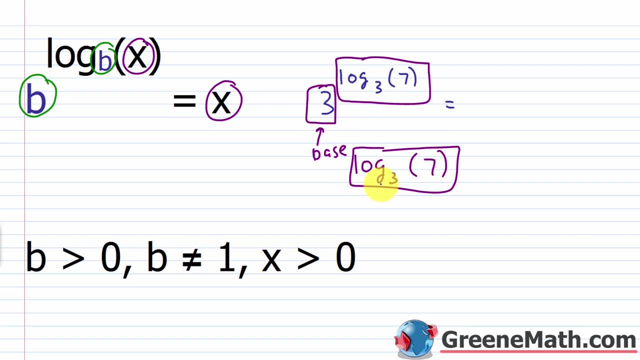 is the exponent that 3 must be raised to to obtain 7.. So, whatever that value is, it doesn't matter. 3 is being raised to it, so I'm going to obtain 7, right? It comes from the fact that the base here and the base here 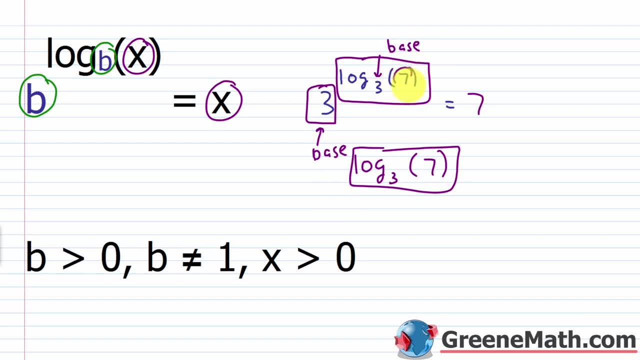 those are the same. So that allows us to just take this value right here, the argument in the logarithm, and just say that's going to be our answer here If I had 7 raised to the power of log base 7 of, let's say, 30.. 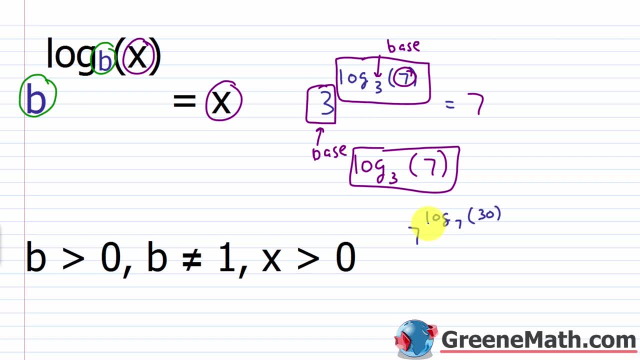 Well, again, this is really easy. 7 is being raised to what? Well, log base 7 of 30 is the exponent 7 must be raised to to obtain 30. So 7 is being raised to that value. so I'm going to get this right here. 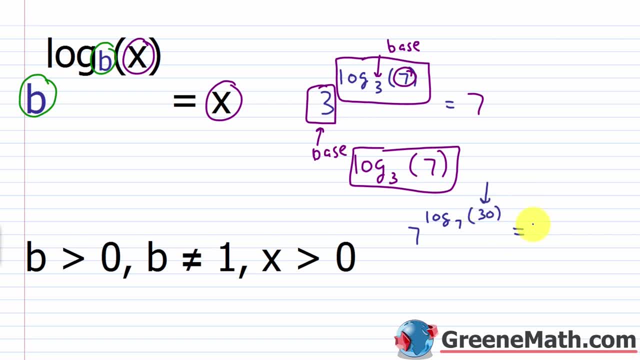 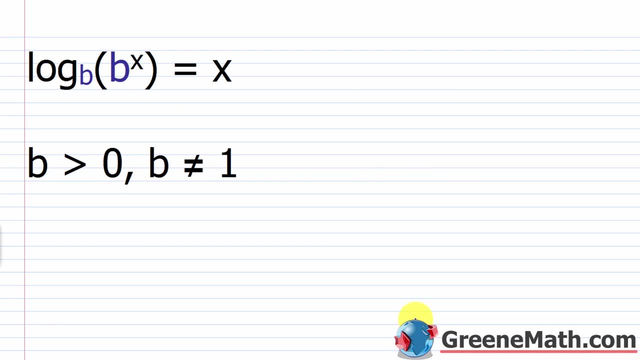 Again the argument in the logarithm, the 30,. so that's going to be my result. All right, let's look at another special property. This is another one that's going to be a time saver for you if you can identify it. 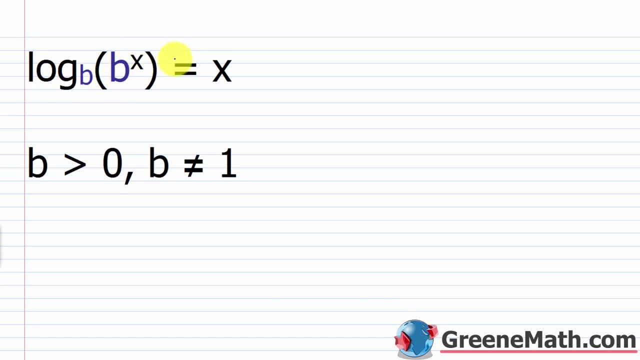 So you have log base p of b to the x is equal to x. The restrictions here would be that b is greater than 0, and b is not allowed to be equal to 1.. Now for this one. it's something you just need to identify. 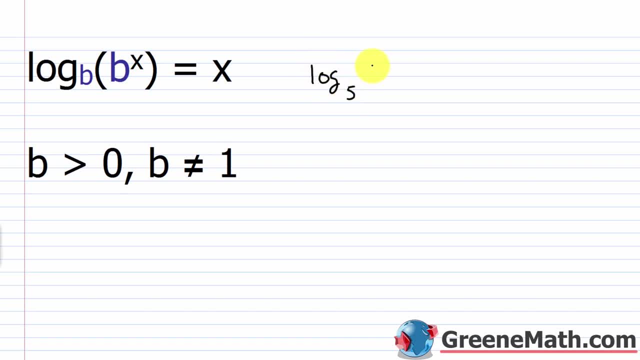 You might see something like log base: 5 of 5 squared is equal to 1.. Well, again, you can kind of pattern match and say: okay, well, there's a b here and a 5 here, So this guy right here would be this guy right here. 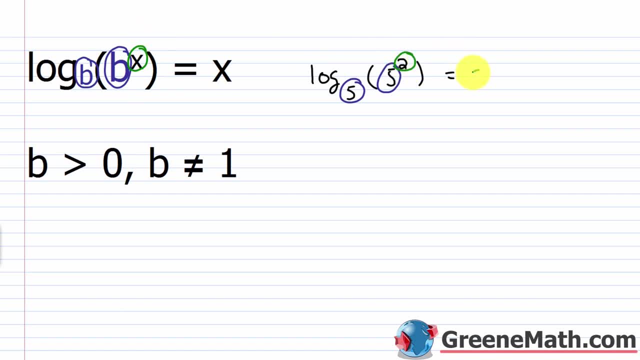 And so my answer is: this guy right here It's the exponent, So the base here- and kind of you think about 5 squared 5 is the base there in that exponential expression. So those bases are really the same. So what I'm saying is that 5 raised to the power of 2. 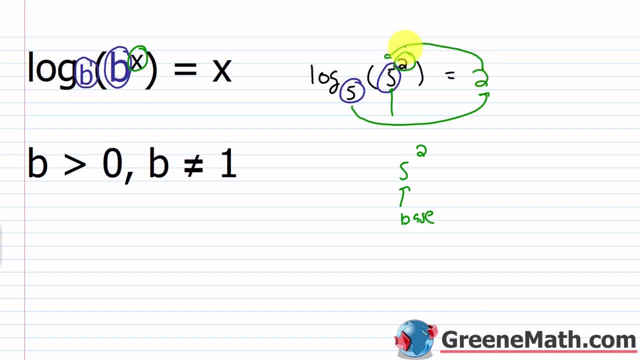 would give me 5 raised to the power of 2, or 5 squared. That's all that's really doing. It's not very complicated to figure that one out If I had log base 9 of, let's say, 9 cubed. 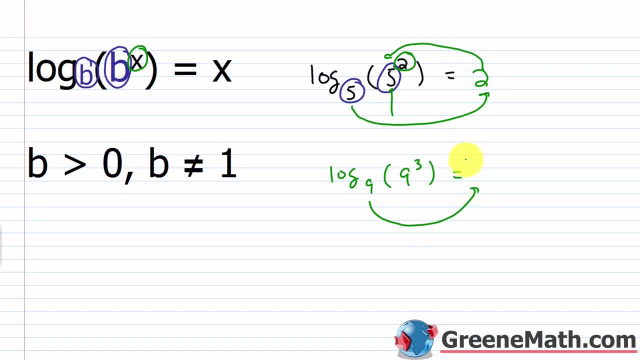 this would be equal to what? 9 to what power would give me 9 cubed, Well, 3.. It's always going to be the exponent as the answer there, because the base here and again, when you think about 9 cubed. 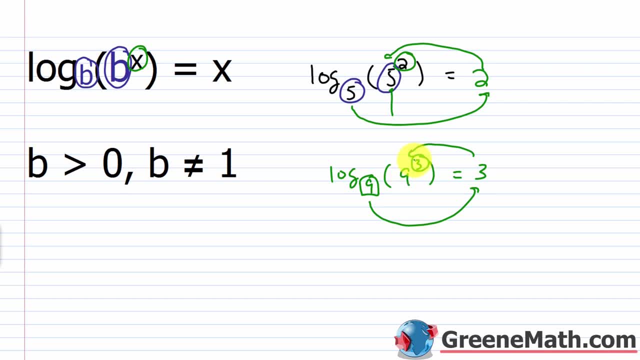 9 is the base there, So those two are the same. So really, I'm just using the exponent as the answer. Okay, very, very simple Now where you might have to think a little bit. you see this on a test. 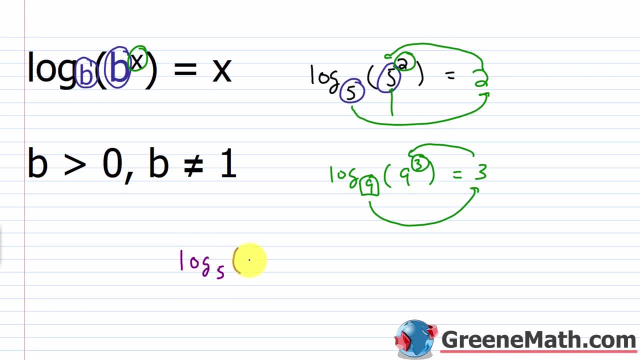 Let's say you got log base 5 of 25, and you want to quickly figure this out. Well, 25, you should know, is 5 squared. So the trick there is to rewrite this as log base: 5 of 5 squared. 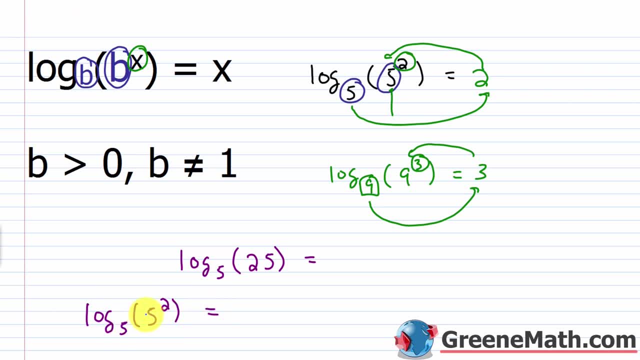 and then you can quickly identify that, hey, 5 here and 5 here are the same. so I know the result here is going to be 2.. Right 5 to the second power would give me 5 squared or 25.. 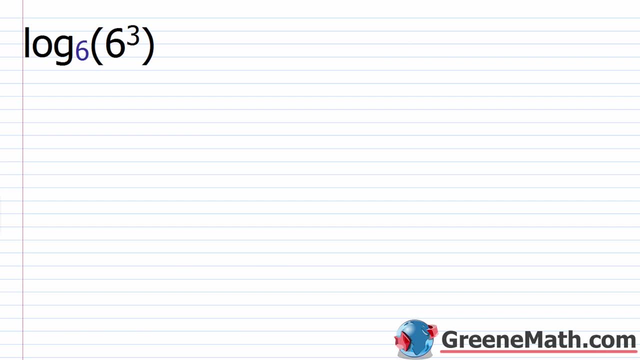 So let's take a look at some examples. We have log base 6 of 6, 6 cubed. So again, this part right here is the same as this part right here. So in other words, 6 to what power would give me 6 cubed? 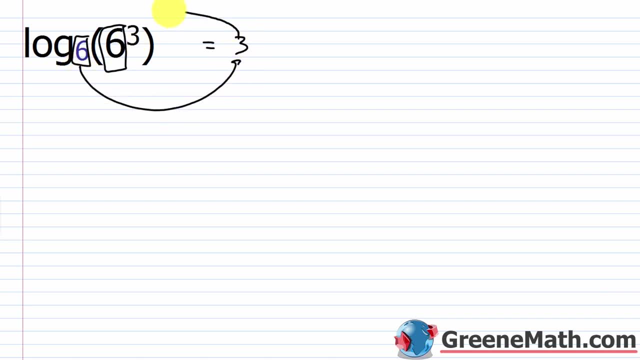 Well, it would be 3.. Right, 6 to the third power would give me 6 to the third power, 6 cubed Log base, 2 of 2 to the seventh power. again, this part right here and this part right here is the same. 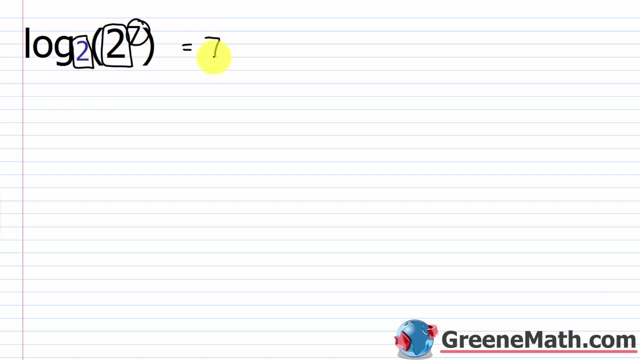 so the answer is just the exponent right there. It's just going to be the 7.. 2 to what power would give me 2 to the seventh power? It would just be a 7.. What about 3 raised to the power of log base 3 of 8?? 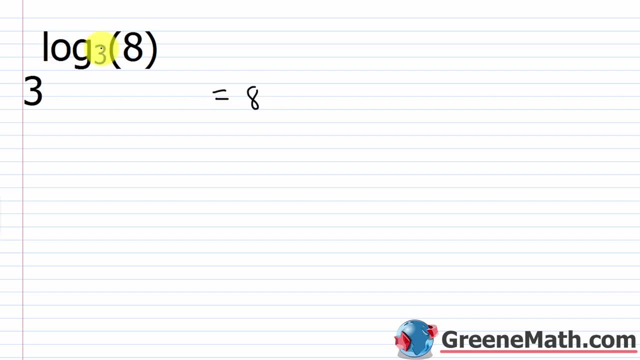 Well, this would just be 8.. Again, this logarithm that's the exponent here, is the exponent to which 3 must be raised to to obtain 8.. So if I raise 3 to that value, I'm going to get 8 as a result. 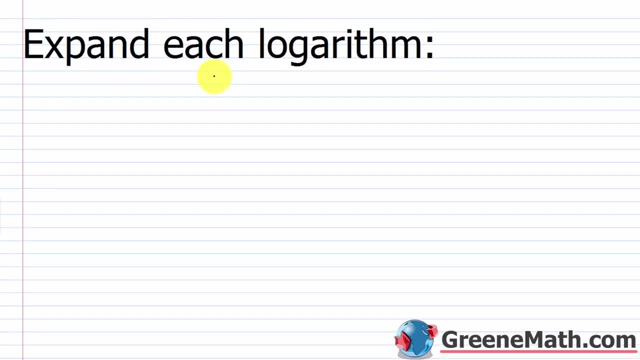 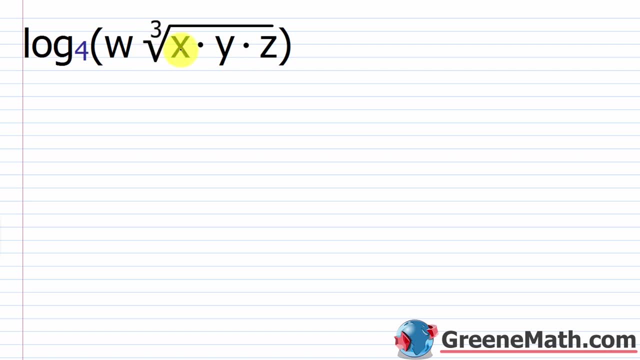 All right, let's take a look at some practice problems. So we want to expand each logarithm. All right, for the first one. we're going to look at log base 4 of. we have w times, the cube root of x times y times z. 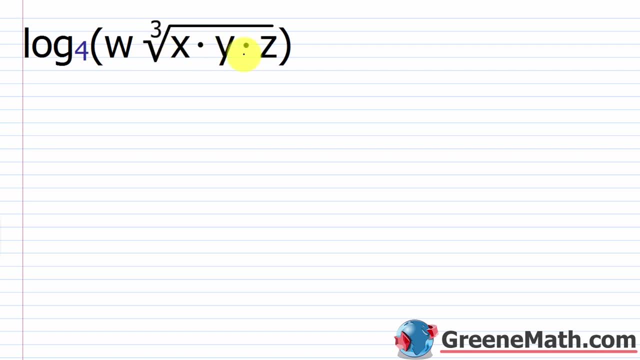 So a lot of ways to kind of attack the problem here. but one way you could do it we could say: this is log base 4 of w plus. remember, this is multiplication here, so it allows you to use the plus symbol. So we'll have log base 4 of this guy right here. 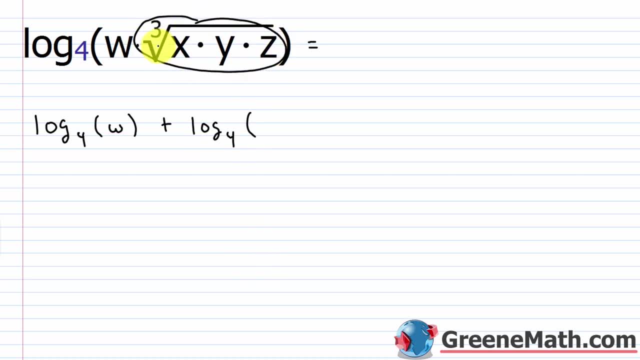 So I'm going to use a fractional exponent here. The cube root of something is like raising it to the one third power, So x times y times z to the power of one third. Now I'm going to take this one third and I'm going to individually raise those factors to that power. 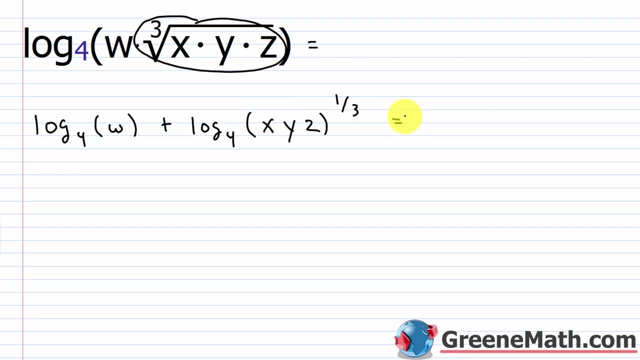 So in my next step I'm going to say this is log base 4 of w, plus log base 4 of x to the power of one third, y to the power of one third, z to the power of one third. Okay, 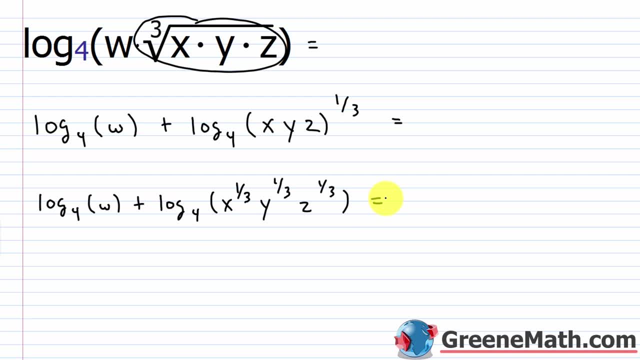 So now in my next step I'm going to use the multiplication here to kind of further expand this part. So we'll say: this is log base 4 of w plus log base 4 of x to the power of one third, plus log base 4 of y to the power of one third. 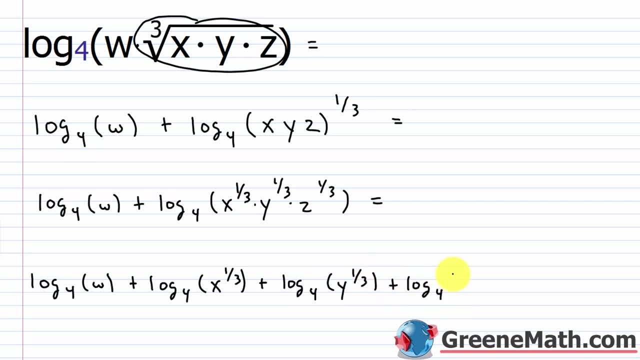 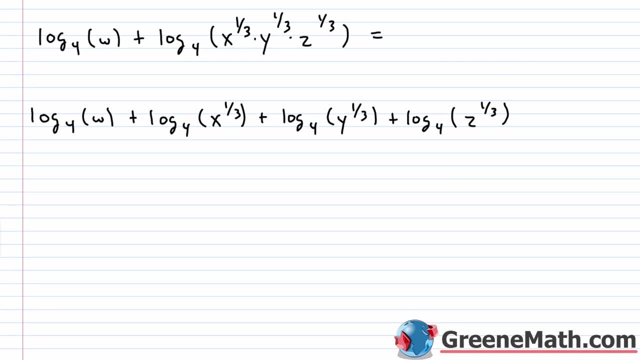 and then plus log base 4 of z to the power of one third. Now the last thing I want to do here, I want to use my power rule and I want to think about these exponents here. Remember, I can write those out in front. 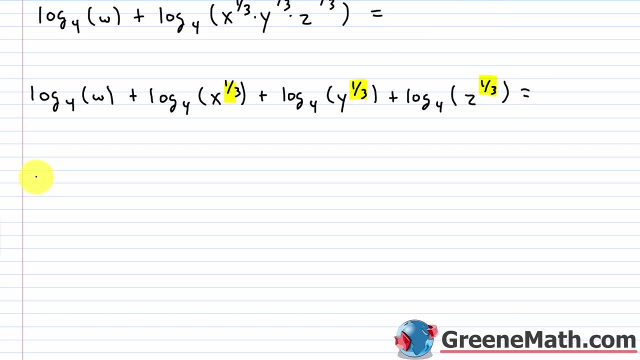 So what I'm going to do is I'm going to say this is log base 4 of w plus this guy's going to come down. so we'll say one third times: log base 4 of x plus this guy's going to come down. 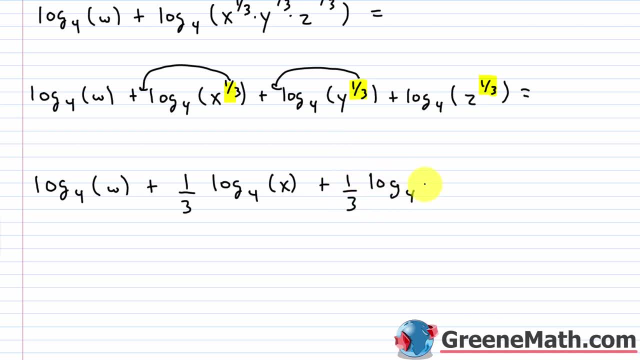 so one third times log base 4 of y, then plus this guy's going to come down, so I'm going to say one third times log base 4 of z. So my answer here is log base 4 of w plus one third log base 4 of x. 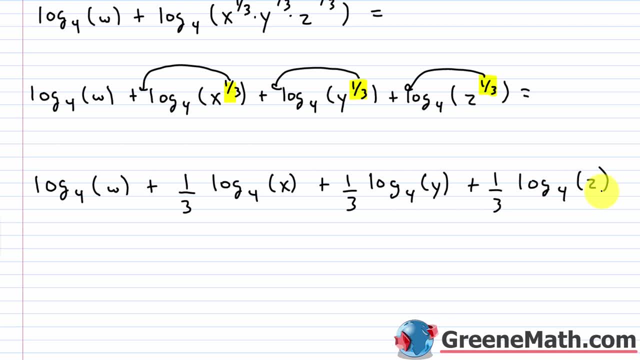 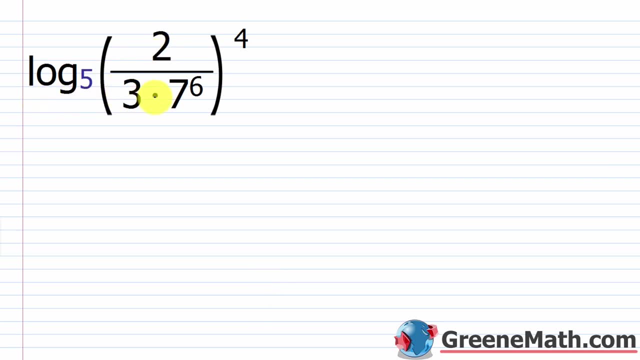 plus one third log base 4 of y, plus one third log base 4 of z. All right, For the next one. we have log base 5 of. we have 2 over 3 times 7 to the sixth power. This is all raised to the fourth power. 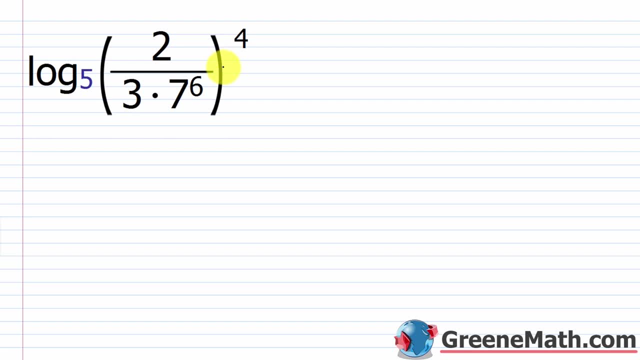 So the very first thing I'm going to do is I'm going to raise everything inside the parentheses to the fourth power. I'm just going to get rid of this exponent here. So this is log base 5 of 2 to the fourth power. 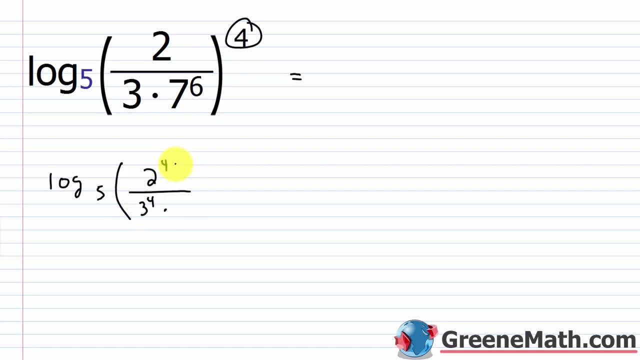 over 3 to the fourth power times. power to power rule. here 7 would stay the same. 6 times 4 would be 24.. Now how do I work with this? You have a division inside of here, So remember the numerator here is going to go first. 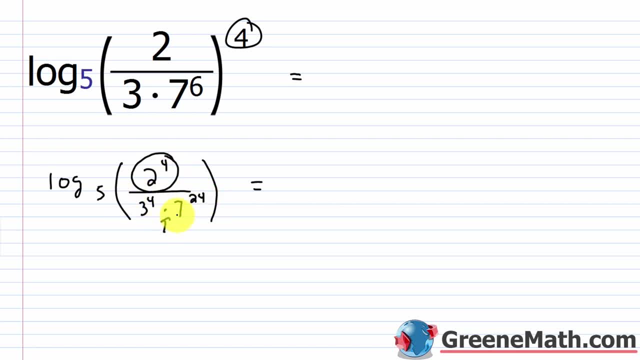 The denominator here has additional multiplication in it. So the way you want to think about this, you have to use parentheses, okay? So let me kind of set this up for you. You have log base 5 of 2 to the fourth power. 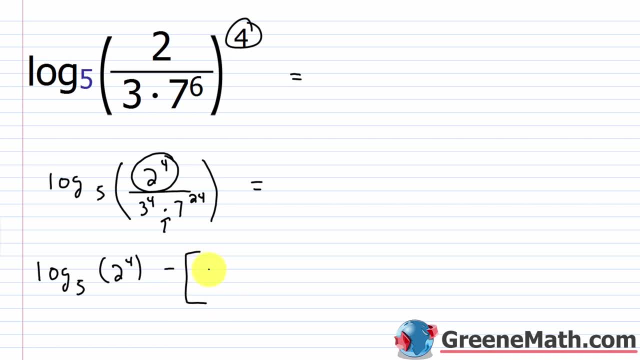 minus. I'm going to use parentheses here. you're going to have log base 5 of 3 to the fourth power plus, because of that multiplication there, log base 5 of 7 to the 24th power. Now, why am I using parentheses? 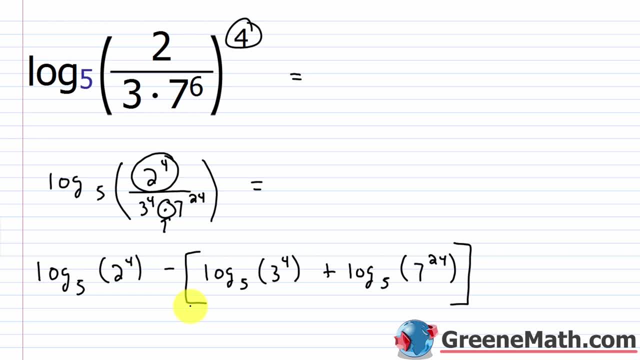 Or, in this case, they're actually brackets. just I'm referring to any grouping symbols that you're going to use. But why am I using brackets here? Well, I'm using that because I want to subtract away this whole thing, right? 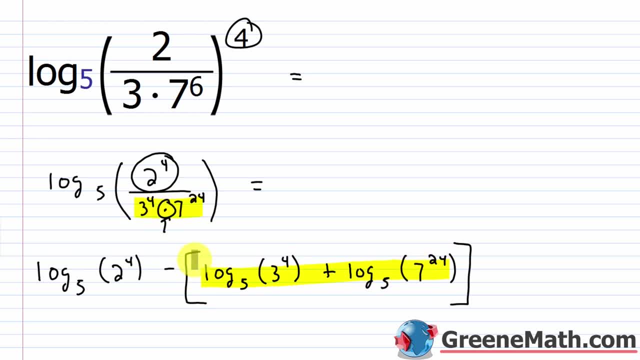 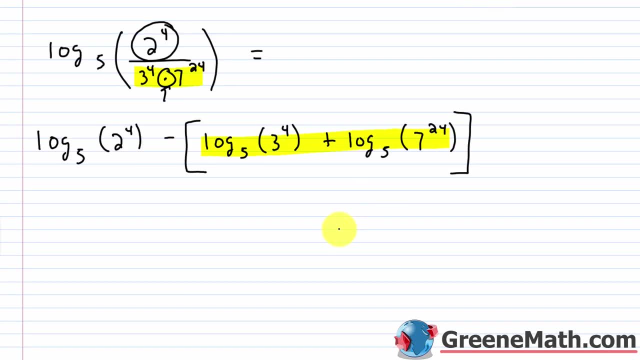 This is from my denominator, So I want to subtract away the whole thing. So I've got to use brackets or parentheses or any grouping symbols that you can kind of think of. All right, So the next step: here we just put equals. 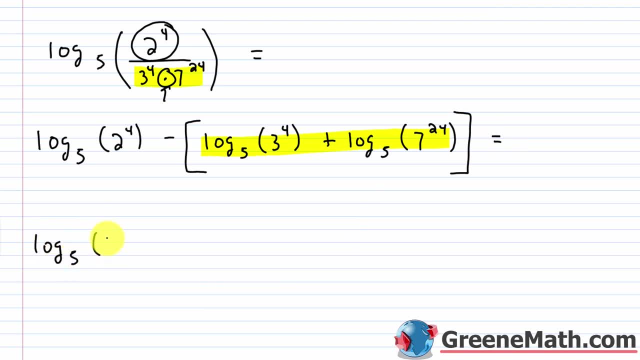 We have log base 5 of 2 to the fourth power, Then minus you'll have log base 5 of 3 to the fourth power. Then this minus would be distributed to this. So we just say minus log base 5 of 7 to the 24th power. 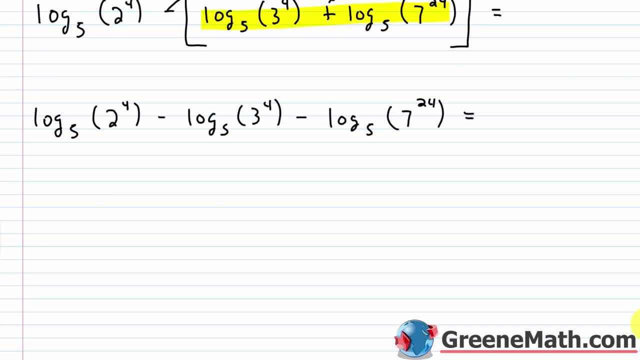 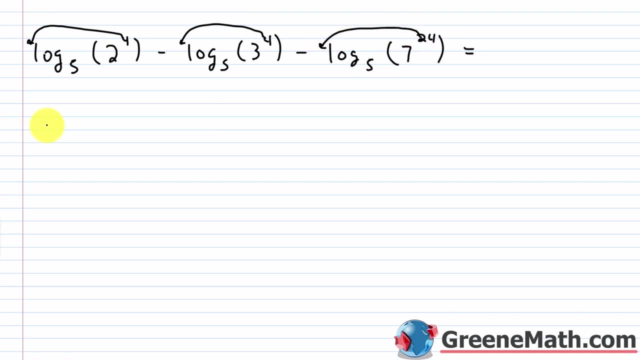 All right. So now let's kind of scroll down and get a little bit more room going. We're going to bring our exponents down in front of each one of these, So we'll have 4 times log base 5 of 2 minus 4 times log base 5 of 3 minus 24 times log base 5 of 7.. 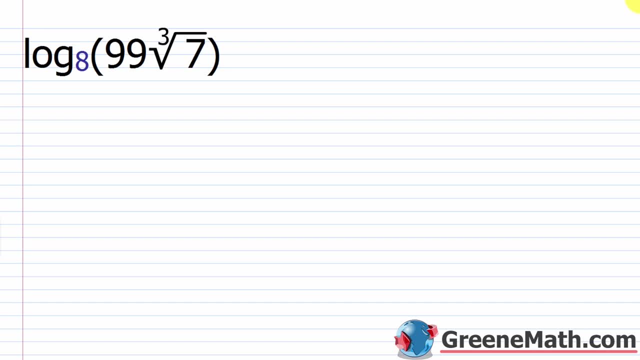 All right, Let's take a look at a note. So we have log base 8 of 99 times the cube root of 7.. So again, I'll say this is log base 8 of 99 plus All right, I have multiplication there. 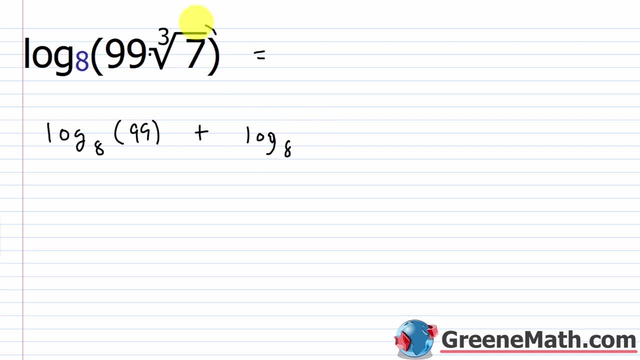 Log base 8 of This guy. right here I would write with a fractional exponent. So I would say: this is 7 raised to the one-third power. Now I want to bring this guy out in front. So let's say this is log base 8 of 99. 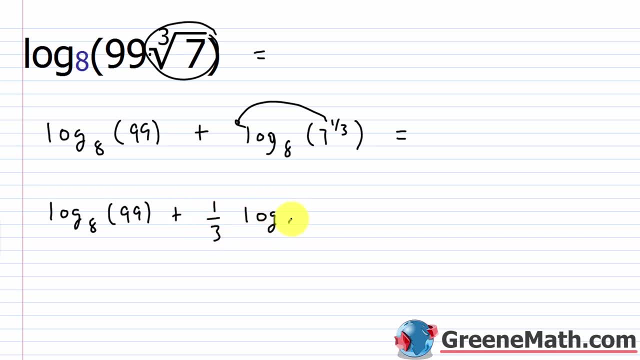 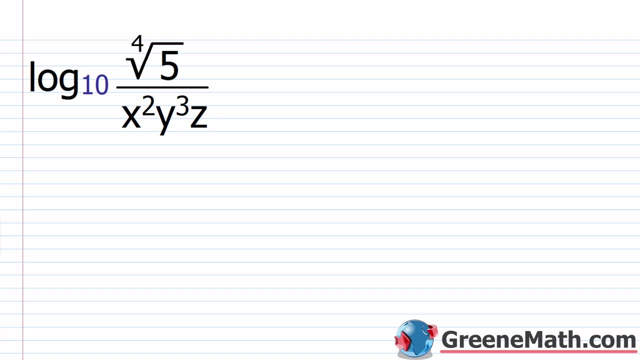 plus one-third times log base 8 of 7.. All right, Let's take a look at another one. So we have log base 10 of the fourth root of 5 over x squared y cubed z. So again I think about log base 10 of the fourth root of 5.. 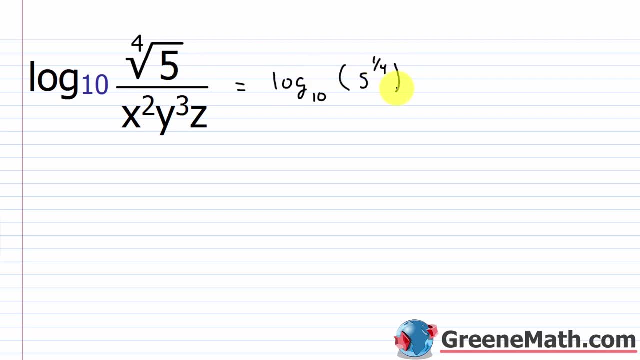 I could write as: 5 raised to the one-fourth power, Then minus I'm subtracting away all this. So I've got to use again some grouping symbols, Parentheses, brackets, whatever you want to use. So let's just do brackets. 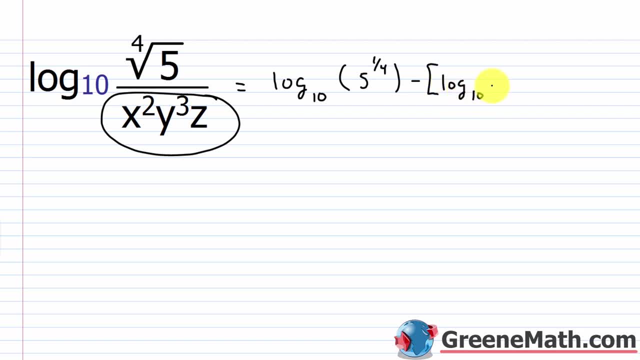 You will have log base 10 of x squared And then you'll have plus- Let me kind of scooch this down so I'm not going to have enough room- So plus log base 10 of y cubed And then plus log base 10 of y squared. 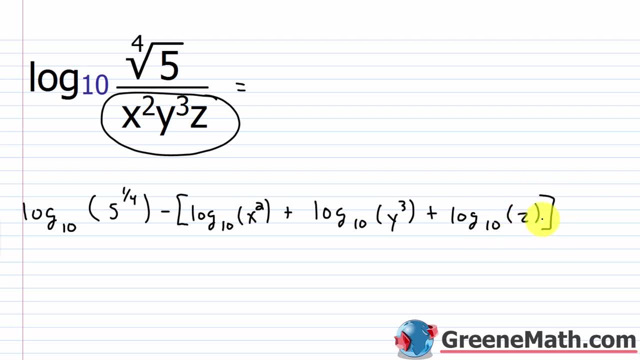 And then plus log base 10 of z, And the grouping symbols are just reminding you to distribute that negative to each term. So if I keep simplifying here, I'll have log base 10 of 5 to the one-fourth power minus. 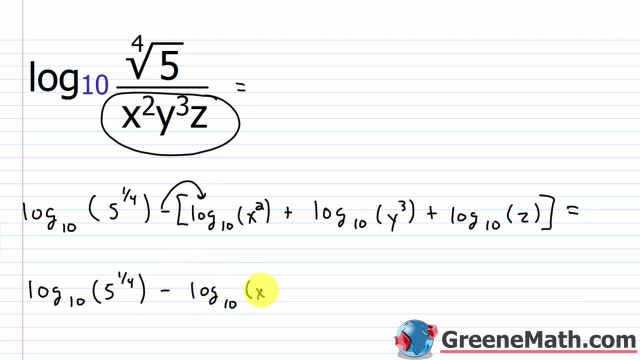 This will go over here. Log base 10 of x, squared minus. log base 10 of y, cubed minus Minus log base 10 of z. Okay, Let's scroll down a little bit. Get a little room going, So let me make that 3 a little bit better. 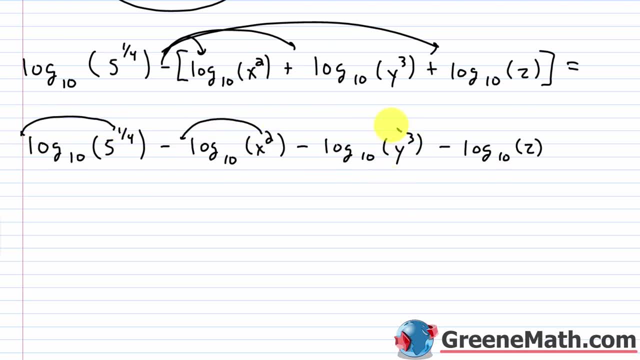 And I'm going to bring all these out in front, So that that and that. So we'll say this is one-fourth times log base 10 of 5, minus 2 times log base 10 of x, Minus 3 times log base 10 of x. 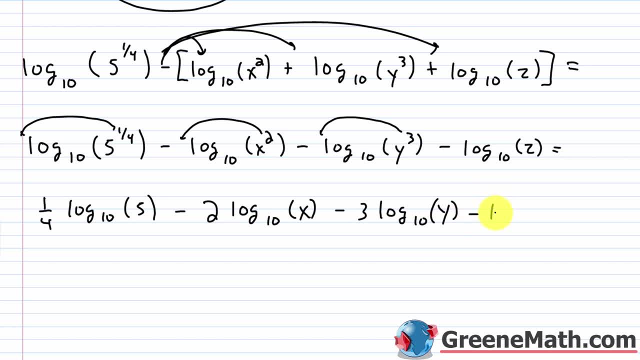 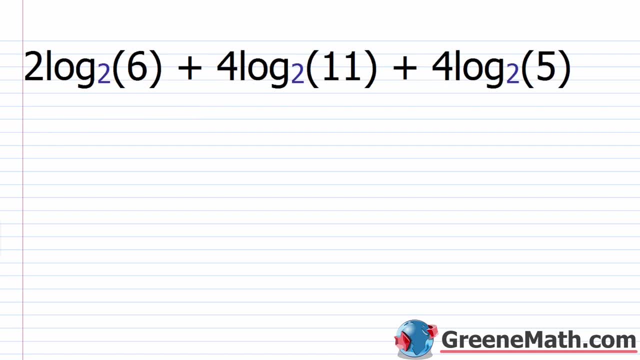 Minus 3 times log base 10 of y And then minus log base 10 of z. All right, So now we want to condense each to a single logarithm. So we have 2 times log base 2 of 6, plus 4 times log base 2 of 11, plus 4 times log base 2 of 5.. 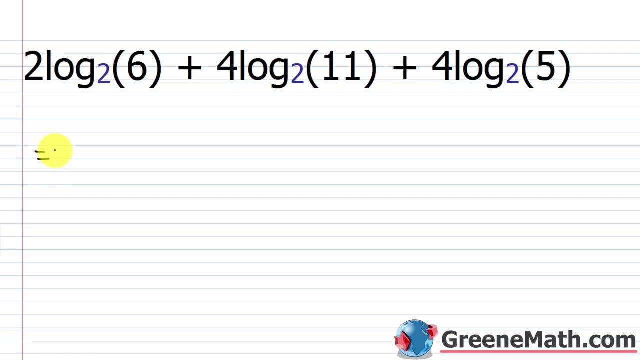 So we're kind of undoing these properties. we just used to expand things. So the first thing is I know that if I have 2 times log base 2 of 6, I could write this as log base 2 of 6 squared. 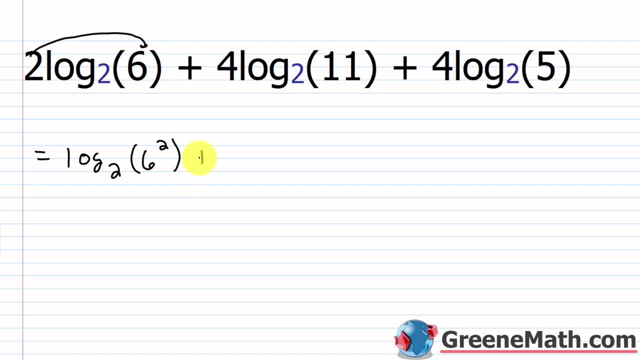 All right, So this would just go back up here. Then plus, if I have the 4 out in front, I know I could write it as up here. So log base 2 of 11 to the fourth power And then plus this guy could go up here. 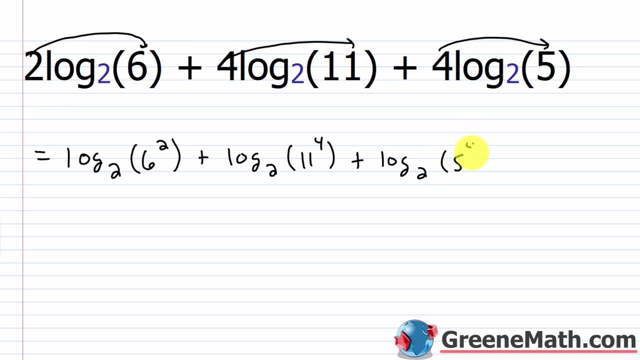 So log base 2 of 5 to the fourth power. Now I have addition, So addition, you go back to multiplication, So everything is log base 2 here, Right? So in other words, it's just going to be log base 2.. 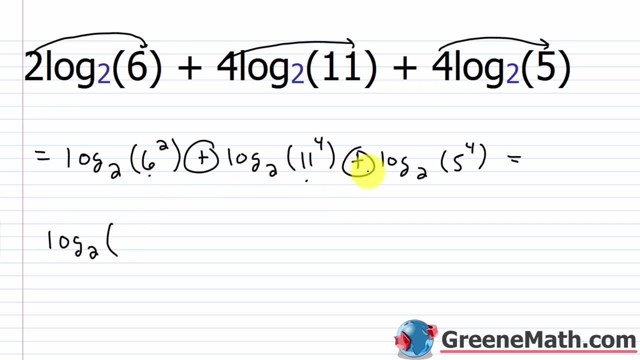 So log base 2 of this guy times this guy times this guy. So 6 squared times 11 to the fourth power times 5 to the fourth power. So in most cases on a test or your homework, this answer is good enough. 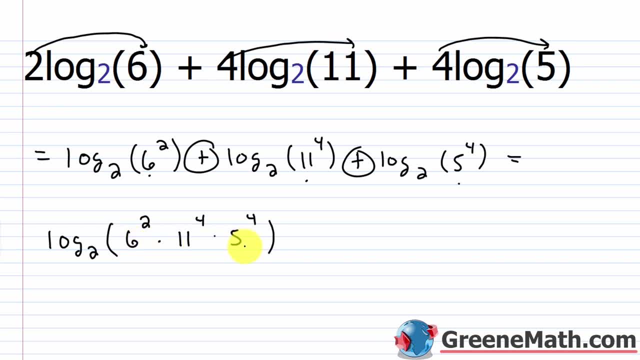 I realized that we could multiply all this stuff together, It'd be a really big number. We're just proving that we can kind of move back and forth. If you wanted to do it, your answer would be 329,422,500. 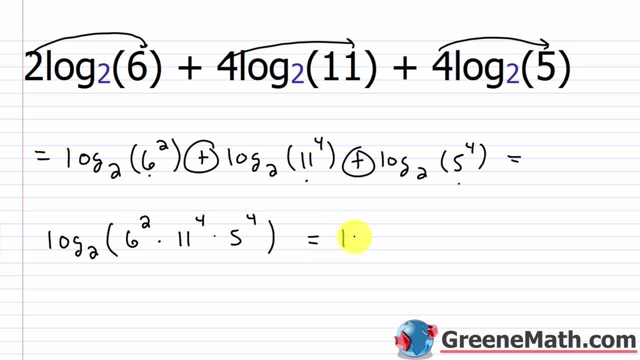 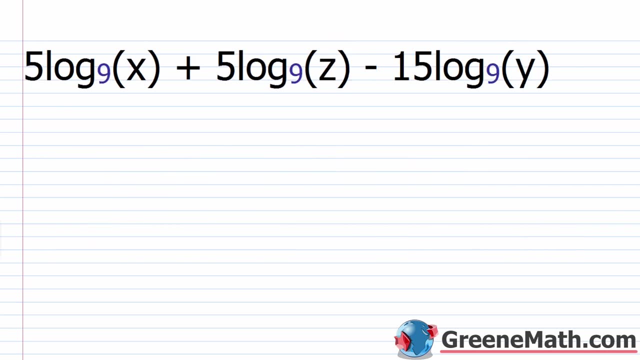 So log base 2 of again 329,422,500.. But again this answer right here is perfectly acceptable. What about 5 times log base 9 of x, plus 5 times log base 9 of z, minus 15 times log base 9 of y? 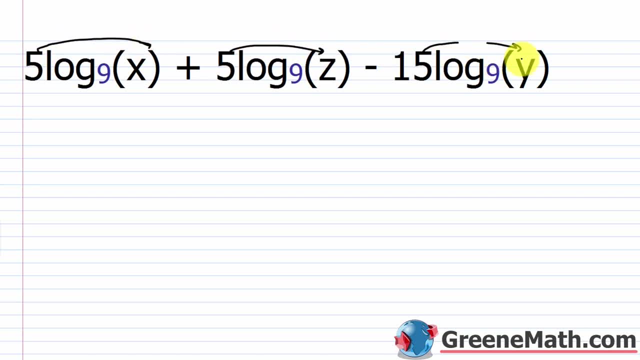 So again, these are all going to go back up here, So we'll do that first. So we'll say: this is log base 9 of x to the fifth power, And then plus log base 9 of z to the fifth power. 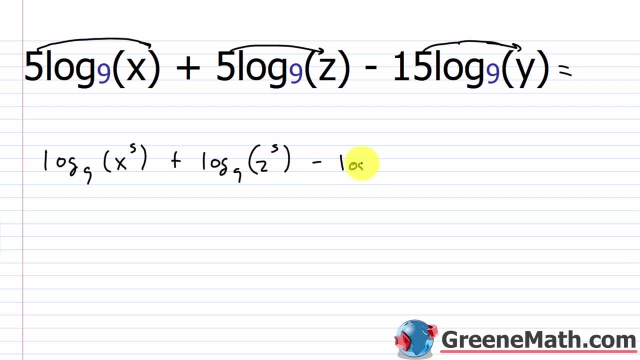 Then minus log base 9 of y to the 15th power. All right. Now the next thing we want to think about is we have log base 9, log base 9, log base 9.. So log base 9 of what? 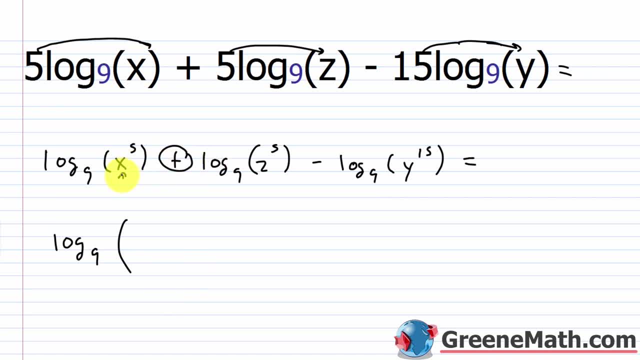 We know these two because there's addition here. This is multiplied by this, So it would be x to the fifth power, times z to the fifth power. Then I have subtraction here. So these two are going to be in the numerator. This guy right here, that's after the subtraction sign, is going to be in the denominator. 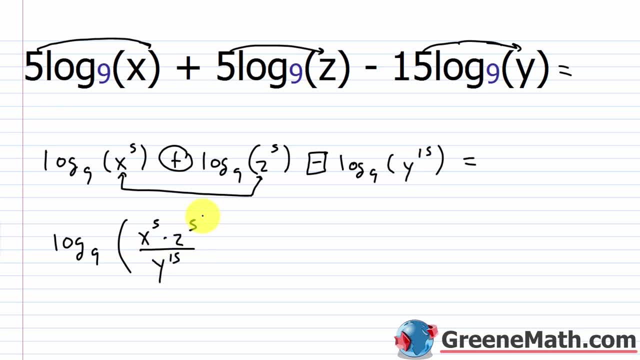 So this is over y to the 15th power. So that's going to be your simplified answer. So log base 9 of x to the fifth power, times z to the fifth power, over y to the 15th power. Let's take a look at one more problem. 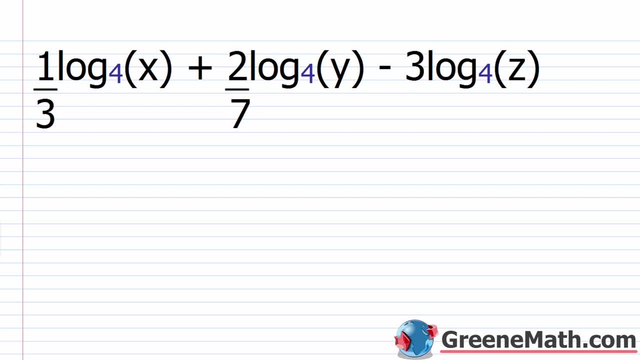 So we have one-third log base 4 of x plus two-sevenths log base 4 of y, minus 3 log base 4 of z. So again, I'm just going to take all these back up real quick And we'll start out with that. 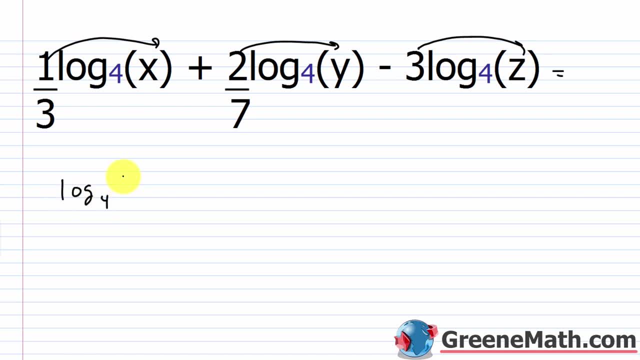 So we'd have log base 4 of x to the one-third power, plus log base 4 of y to the two-sevenths power, minus log base 4 of z to the 15th power. So this equals what? Well, we'll have log base 4 of. 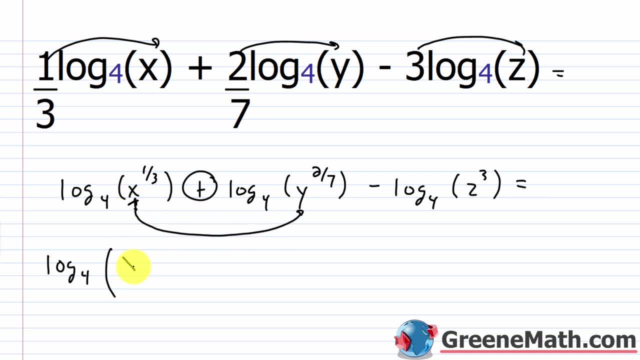 I have my addition here, So this one times this one. So x to the one-third power times, y to the two-sevenths power. So we have this subtraction involved here, And so we know this is going to be over. this z cubed here. 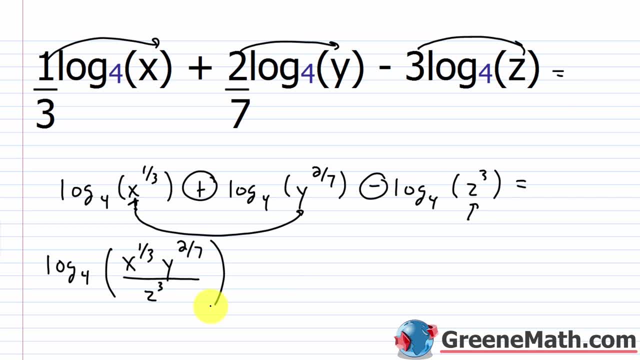 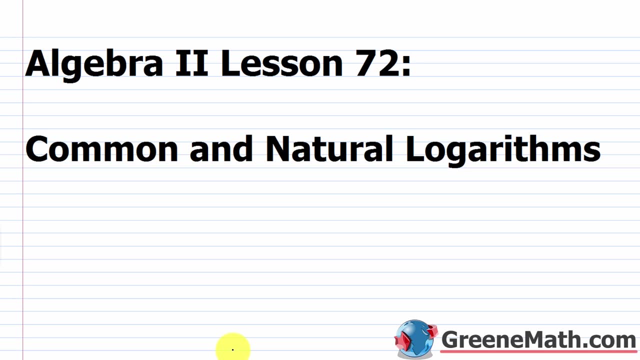 the subtraction. so that's going to come right here. So you end up with log base 4 of x to the one-third power times, y to the two-sevenths power. This is over z cubed. Hello and welcome to Algebra 2, Lesson 72.. In this lesson we're going to learn about common and natural logarithms. So far when 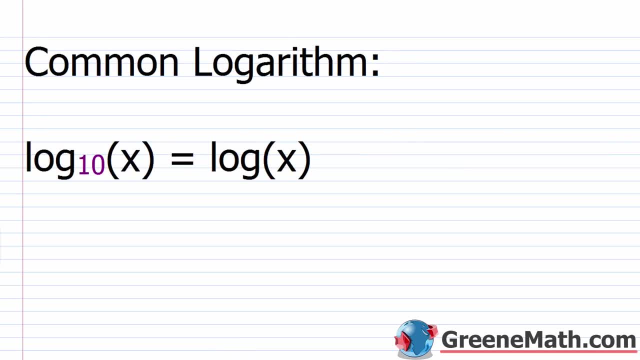 we dealt with logarithms. if we came across a logarithm with a base of 10, we listed the base of 10, just like we would for any other logarithm. But there's a shortcut involved when you see a logarithm with a base of 10.. So a logarithm with a base of 10 is known to us as a common logarithm. 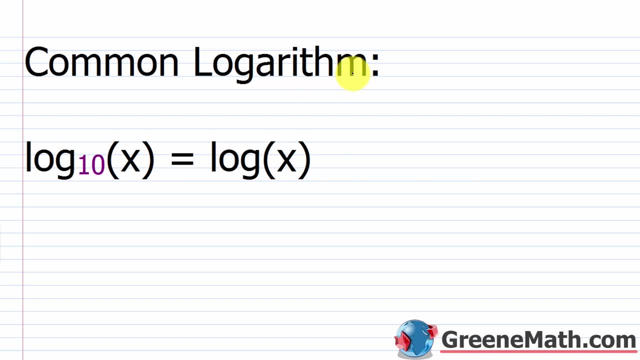 This is because we have a base 10 number system, So when we encounter one of these guys we don't actually have to list the base. So something like log base 10 of x could be written as just log of x, right? So the base here is understood. 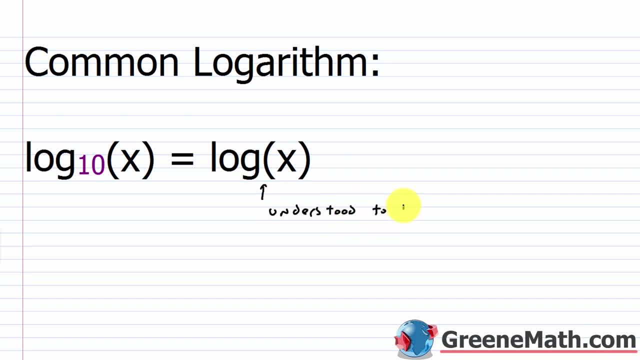 To be 10.. So if I saw something like log of 100, this is understood to have a base of 10.. So this is really log base 10 of 100.. And we all know this is 2, right 10 to the second power will give me. 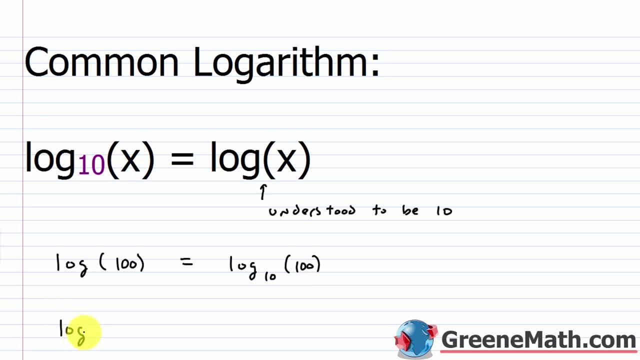 100. Or if I saw something like log of, let's say, 30. We know this is log base 10 of 30. So if you're working with logs and you see log of some number and you're like, what is the base, 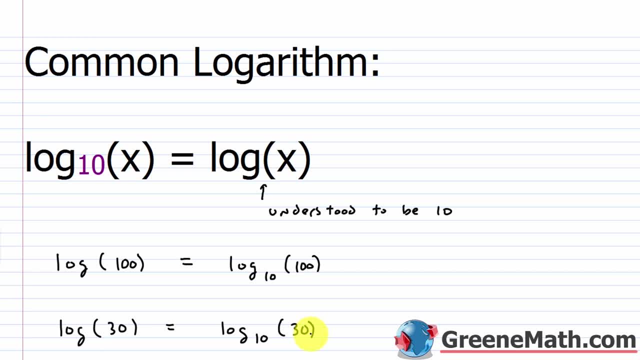 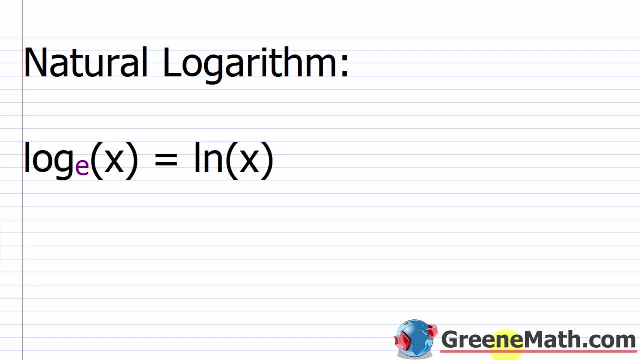 Again. it's just understood to be 10.. You've come across a common logarithm. Now, another important logarithm we're going to come across is known as the natural logarithm. So the natural logarithm obtained its name because of its place in biology and natural situations where growth or decay is. 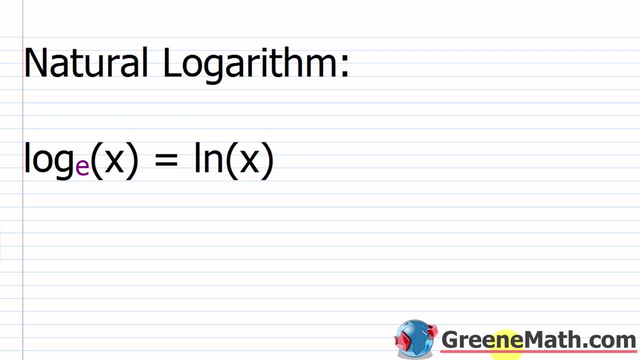 involved. So the natural logarithm has a base of e. So if you see something like log base e of x, this base right here, this is what we're talking about. In e, this number is approximately equal to 2.71.. This e here is going to come up a lot, okay. 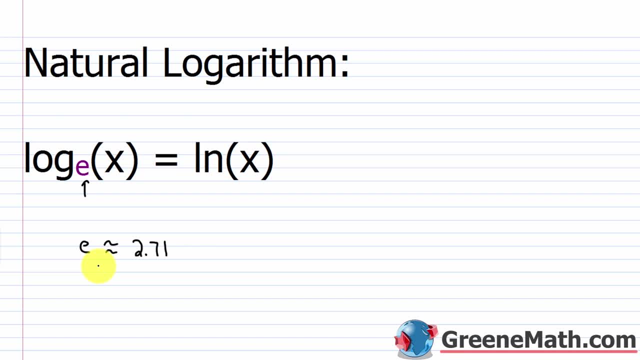 when we're working with math, moving forward, And just think of it as kind of another number that you're going to encounter, like pi. It's this special, irrational number Again after the one here there's an infinite number of digits. There's no pattern to it. It just goes on and on and on. 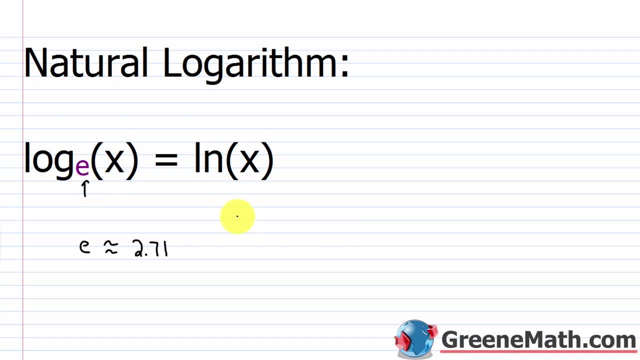 So essentially, what we can do is just find the base. when we have this base e of x, we can use it to calculate the binary, And this is actually going to be a little bit more complicated than what I was talking about last time. When we see log base e of x, we can abbreviate this and 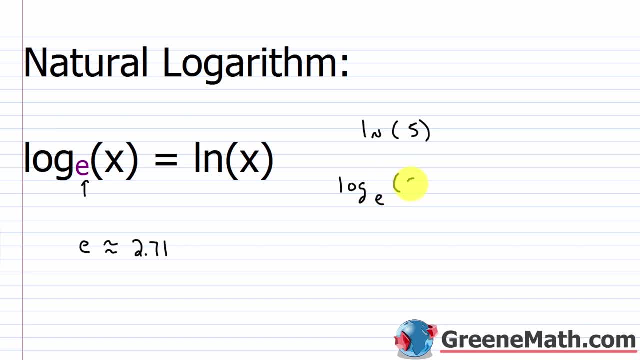 just say this is the same as saying ln, which stands for the natural logarithm of x. So if I see ln of 5, this is the same as saying we have log with a base of e of the number 5.. Okay, these two. 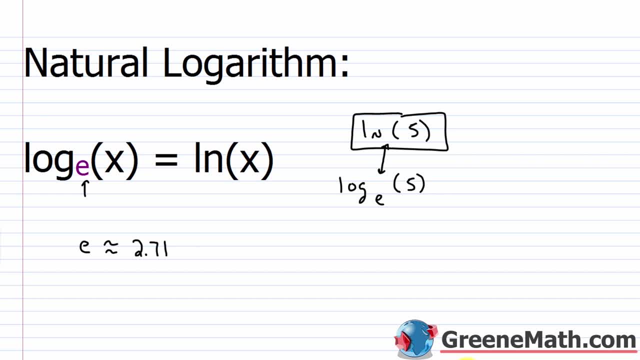 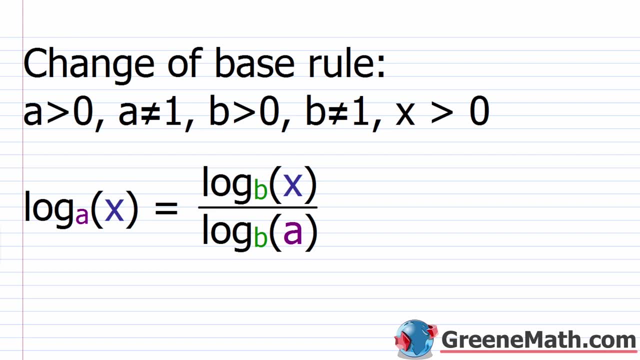 are the same calculator to either get an exact value or an approximate value for a logarithm. So the reason it's important to talk about the common logarithm and the natural logarithm, these are the two buttons that are going to be available to you on most calculators. Now there might be some. 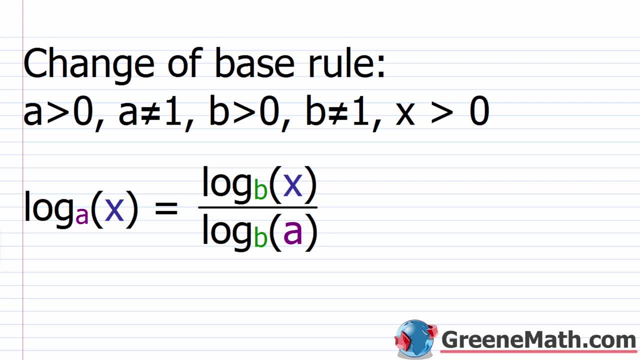 calculators out there that allow you to change the base of a logarithm. The calculator I have, the calculator that most of you will have, gives you just an ln key for the natural log and gives log key which is for a base 10 log or common logarithm. So if you are in that situation, like 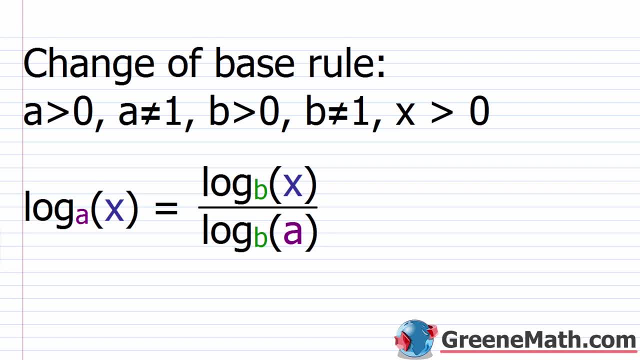 I am. you need to use a change of base rule in order to plug logarithms into the calculator and get either an exact value or, most cases, an approximate value. So the change of base rule goes like this: For a greater than zero, a not equal to one, b is greater than zero, b, not equal. 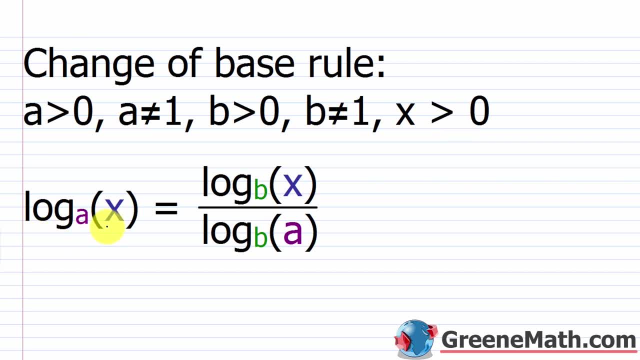 to one and x is greater than zero, you have log base a of x. This is equal to log base a of x, log base b of x over log base b of a. So just notice that the base here and the base here is: 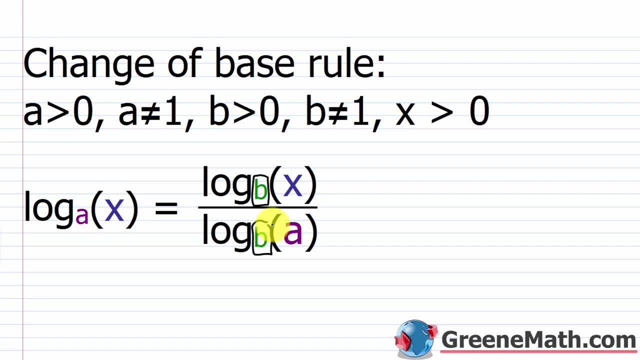 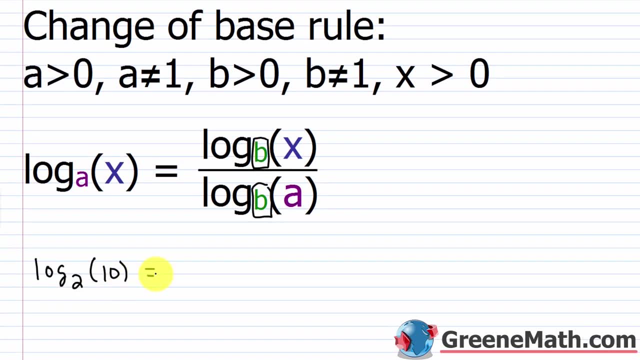 the same. So in most cases we're just going to use the common logarithm. So if I had something like log base 2 of 10, and I wanted to change this to a common logarithm or a base 10 logarithm, 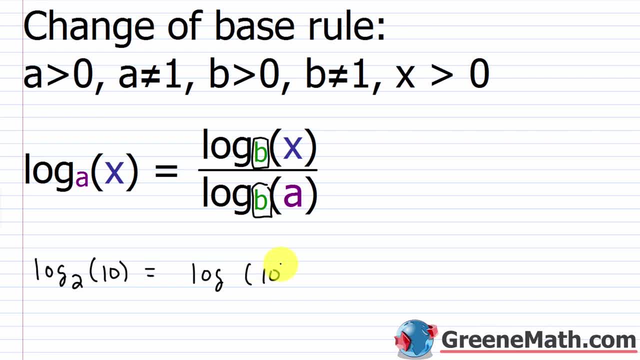 I could just say: okay, well, this is log of 10 over log of 2.. Okay, And you could punch this into your calculator and you could say: okay, well, this is log of 10 over log of 2.. And you: 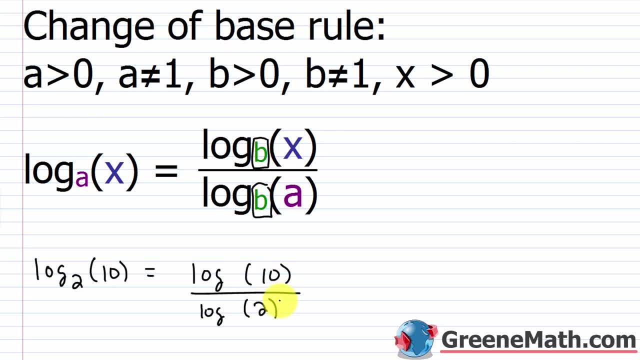 get an approximate value, And if I went to three decimal places on this, I could say this is approximately equal to 3.32.. It's one and then a nine. So the nine allows me to take that one up to a two, and then everything after that would be a zero if I was rounding. So 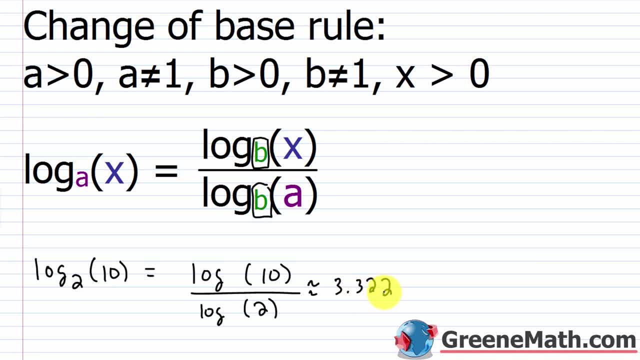 let's just say this is approximately 3.322.. Okay, So, knowing that I couldn't have typed this into most calculators, but I can type this into most calculators and I can get an approximate value, I get this. So that's where the change of base rule comes into play. Again, my base here and my 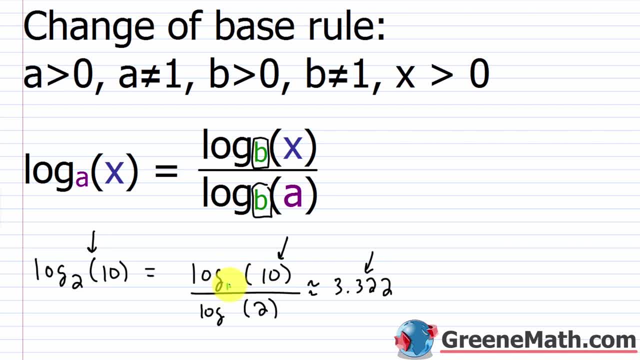 base here are the same. I might as well have just wrote: this is base 10 and base 10.. But again, if I just write log of something, I understand that the base is 10.. So that's why I use that. 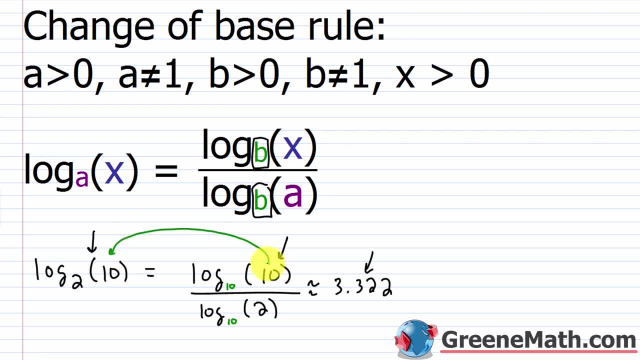 little shortcut. Then this guy right here came from this: Okay, Again, just follow the pattern. This right here, your argument in the logarithm is going to go as the argument in the logarithm in the numerator. Then this right here, the base: 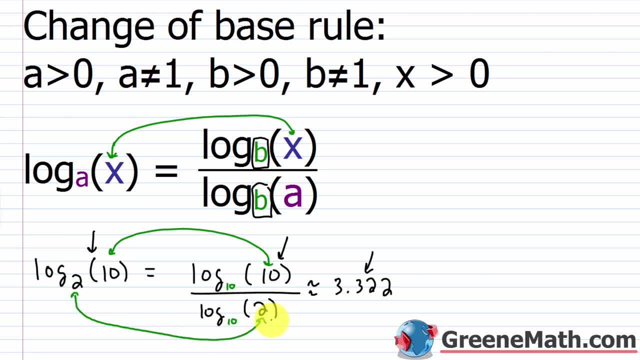 okay, the base is going to become the argument in the logarithm, in the denominator. So just following that pattern you can change the base and you'll be able to key that in to your calculator And you'll get the same result if you use the natural log. So if I said ln of 10, 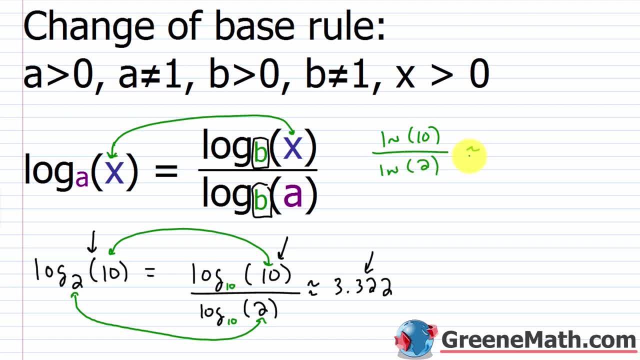 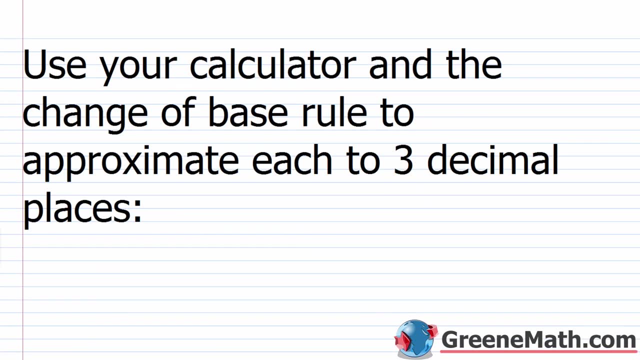 over ln of 2, I would get approximately 3.322 as well. Okay, So same thing. either way, if you want to use the natural log or if you want to use the base 10, log or the common logarithm, it's going to be the same answer, All right. So now we want to use 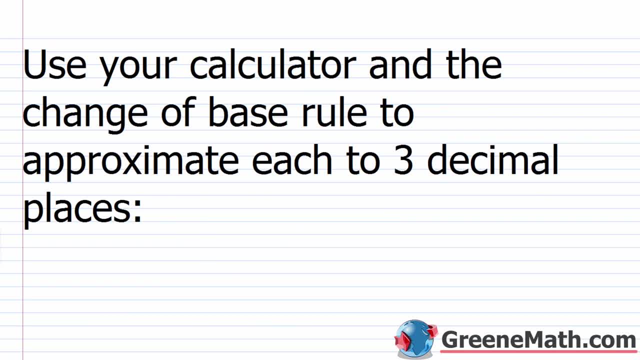 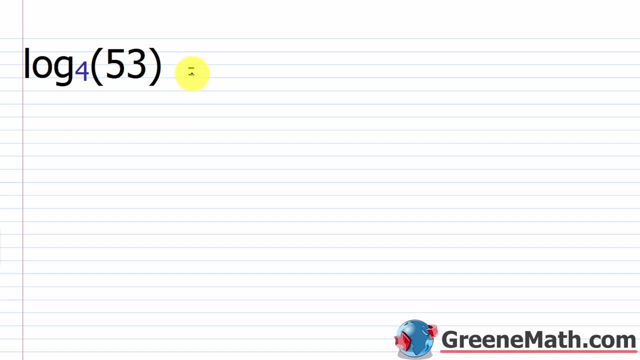 your calculator and the change of base rule to approximate each to three decimal places. All right, So we have log base four of 53. So I'm going to change the base to a base 10 log And so I'm going to say this is log of this guy 53, over log of this guy, which is four. 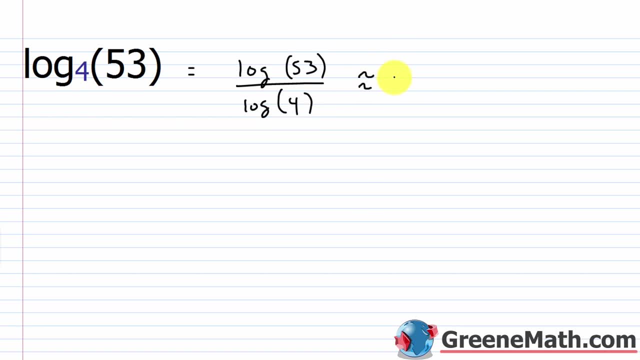 So what's that going to give me? It's approximately what. So my calculator, the readout, gives me 2.863960227.. If I want to approximate each to three decimal places, I'm looking at this guy right here. So here's where I would look and say: okay, well, the nine is in the category of five. 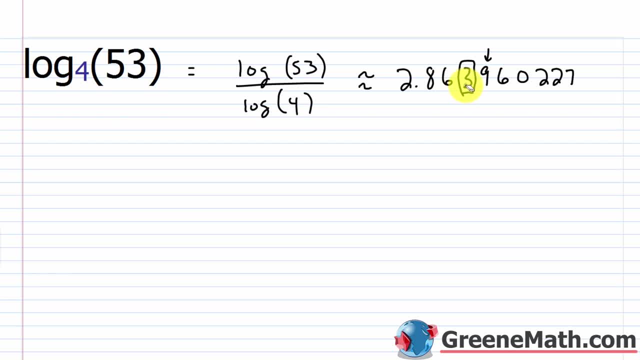 or greater. So I would round up right. So this would turn into a four, And then everything after that would be a zero and I could just cut it off. So I'd end up with approximately 2.864.. What about log base five of 2.864?? 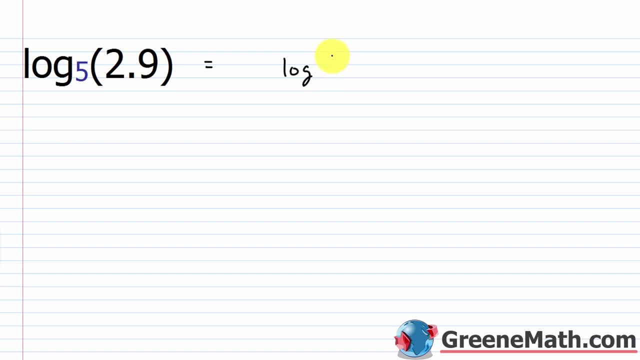 So this would be equal to log of 2.9 over log of five. So this would approximately be what? So my calculator gives me 0.6615419761.. But again, if we're approximating this to three decimal places, well then you've got one, two, three. 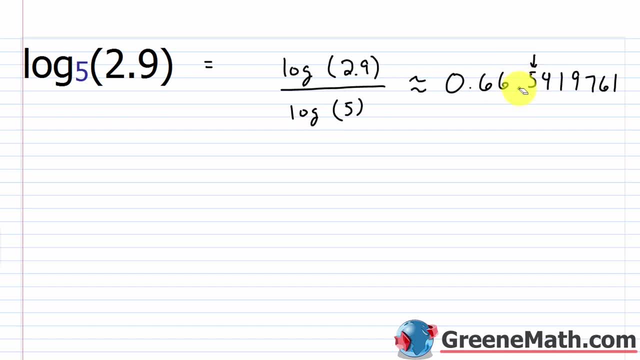 so you're looking there. So the guy after is a five, So I can make this into a two and then I can cut everything else off. So this is approximately 0.662.. All right, now we're looking at log base four of 3.4.. Let's go ahead and just use the natural. 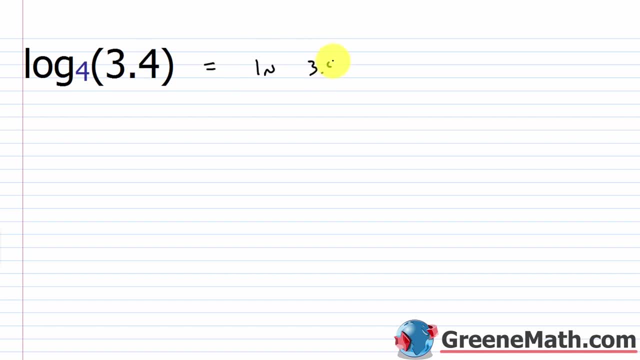 logarithm. So let's do ln of 3.4 over ln of four. So what does this give us? Well, this would approximately be equal to: you've got 0.884.. So we've got 0.884,. so we've got 0.884.. So this is approximately 1.827673732.. 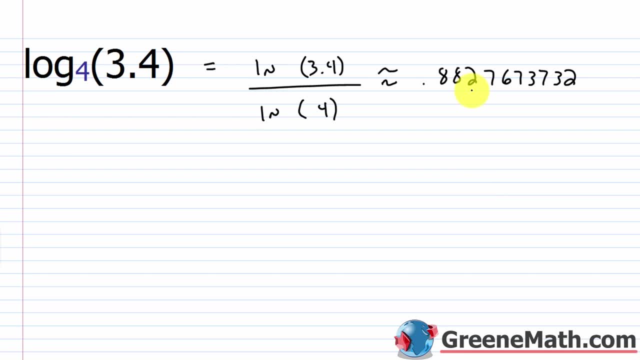 That's the readout I get from my calculator. So for three decimal places I'm looking at that digit there And so the seven here. the digit after is in the category of five or greater. So I can go ahead and round up and say this is a three, and then I can cut everything. 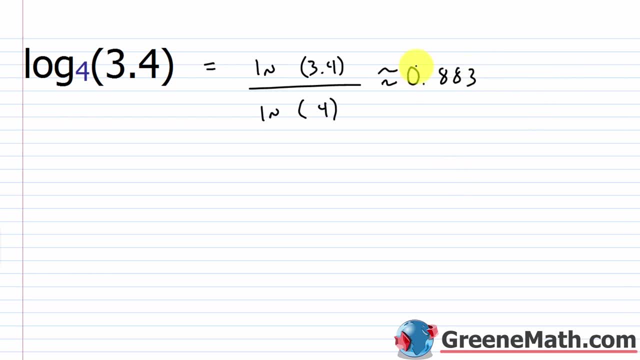 else off. So this is approximately equal to 0.883.. What about log base two of 23?? What do we get there? So I can say that this is a three. I'm going to go ahead and do the So I can say this is log of 23 over log of 2.. 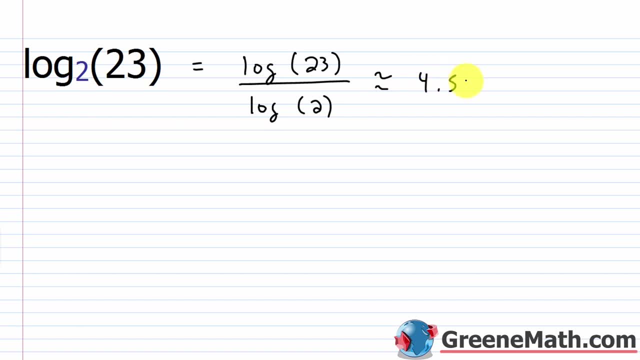 So this is going to be approximately equal to 4.523561956.. So three decimal places right there. Then I'm looking at this digit here. This is in the category of 5 or greater, So I can round up That 3 will become a 4.. 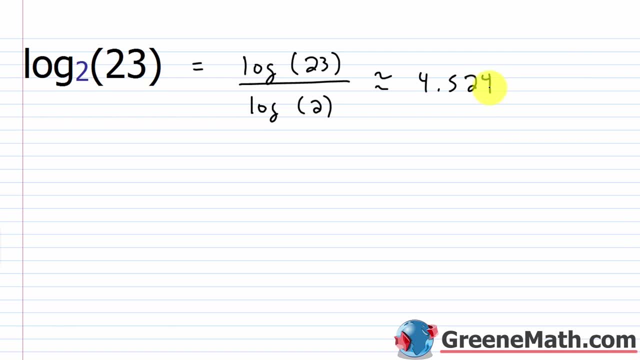 And I can cut everything else off. So this is approximately equal to 4.524.. What about log base 7 of 66?? So let's say this is ln of 66 over ln of 7.. So this will be approximately equal to: you'd have 2.153056627. 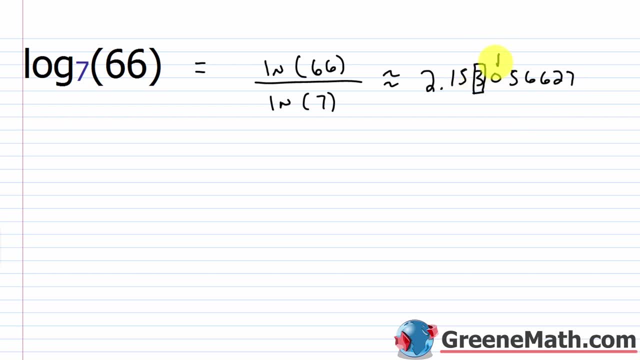 So three decimal places. You're looking at this right here. The 0 that comes after falls in the category of 4 or less. So we would leave the 3 unchanged and we would just cut everything off here. So your approximate answer would be 2.153.. 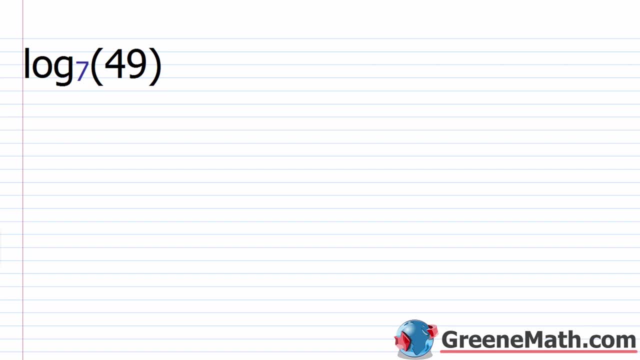 What about log base 7 of 49?? Well, most of us know that that's equal to 2. But let's just for the sake of doing the example here, let's punch this up on a calculator. Let's go log of 49 over log of 7.. 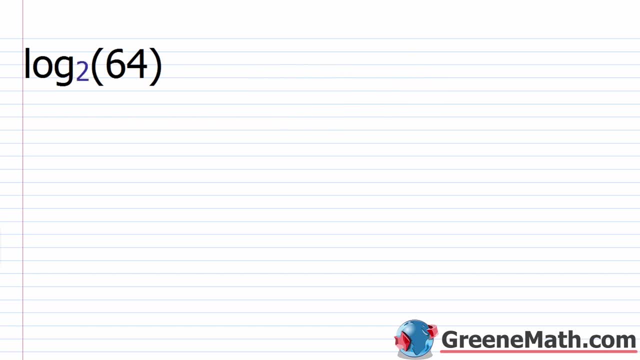 And you'll see that you get an answer of 2, exactly. What about log base 2 of 66?? So this is another one that we can get a perfect answer for. We know that 2 to the 6th power is 64.. 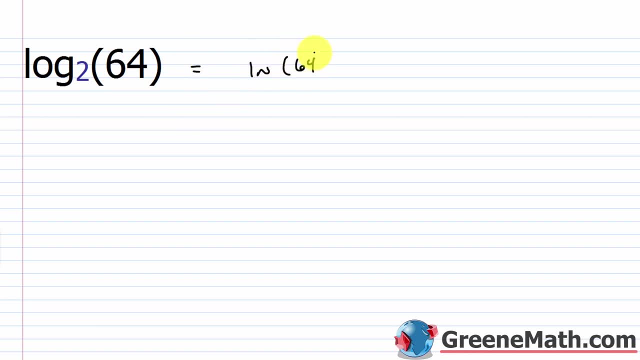 So for this one, punch up on your calculator ln of 64 over ln of 2. And you're going to find that you get an answer of exactly 6.. All right, let's look at one that's a little bit challenging. 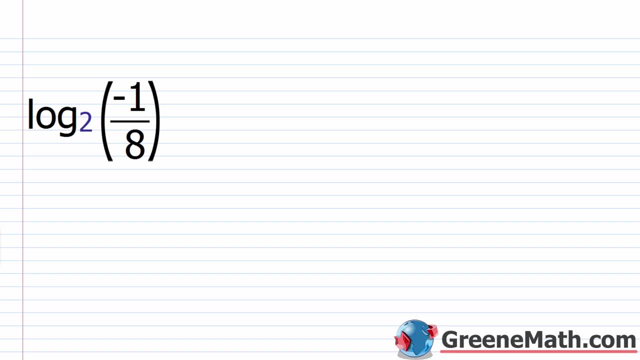 So let's say you get log base 2 of negative 1 8th. Is negative 1 8th allowed to be the argument of a logarithm? No, it is not. Remember we say that this guy right here has to be greater than 0.. 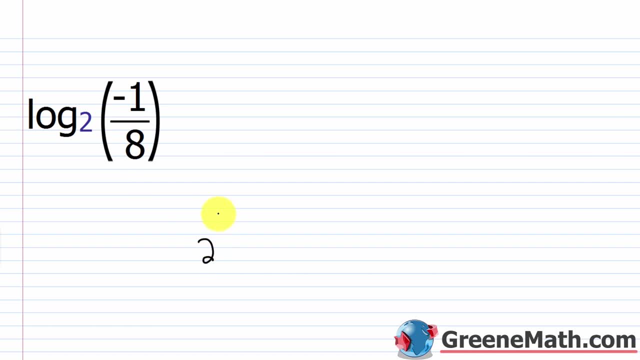 Why is that the case? Think about this for a second: 2 to the power of what would produce negative 1, 8th. You can't do it. If I raise 2 to a positive number, I get a positive number. 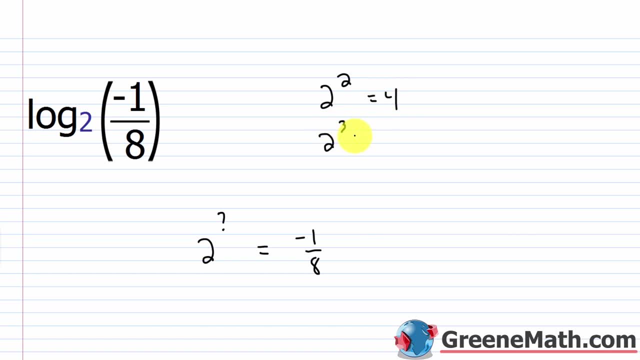 So like 2 squared is 4, or 2 cubed is 8, so on and so forth. If I raise 2 to the power of 0, I get 1.. If I raise 2 to a negative number, so like negative 4,. 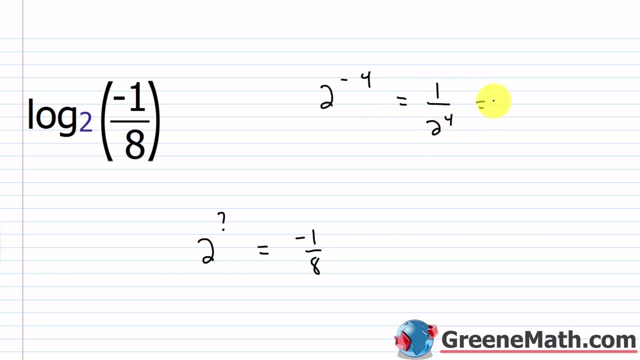 it's 1 over 2 to the 4th power, which is still positive. right, This is 1 over 16.. As this guy gets more and more negative, we're going to get a value that's closer and closer to 0,. 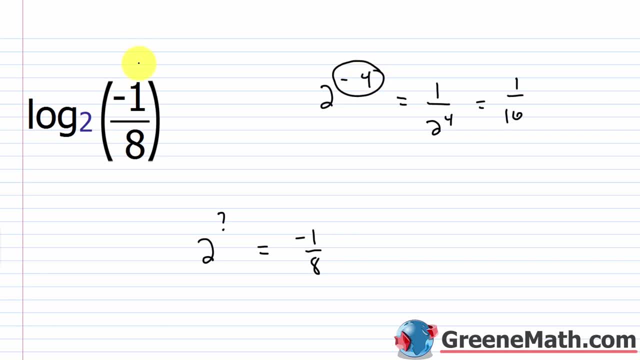 but it will never actually become negative. So this right here is not a possibility for an argument in a logarithm, And so because of that we can say this guy is undefined, right, We don't need to do a change of base rule. 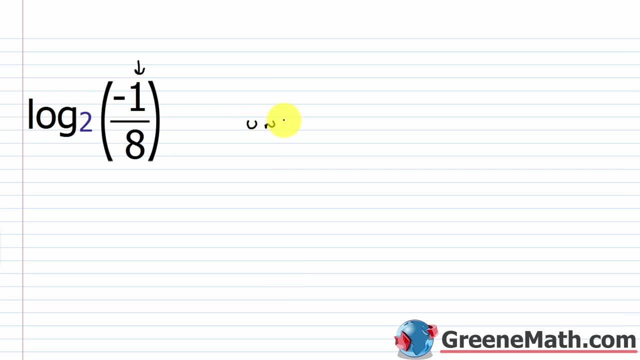 If we see something like this as a trap question, we just say it's undefined. What if we saw log base 2 of 1: 8th? Well, in this scenario, 1, 8th is positive, so we can get an answer here. 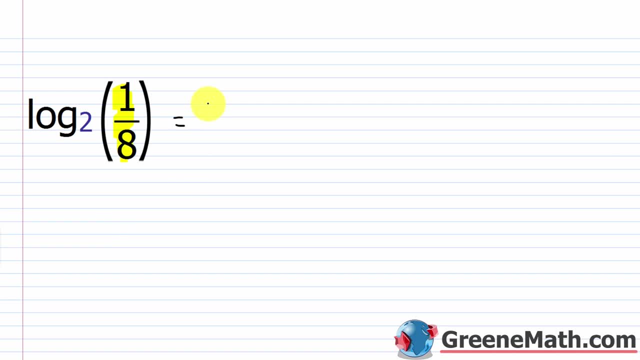 We know that 2 to the power of negative 3 would give me 1- 8th. but again, for the sake of doing this for this exercise, let's just go ahead and say this is log of 1- 8th over log of 2.. Punch that up on your calculator and you should get negative 3.. So we're going to get 1 8th. So we're going to get 1 8th over 1 8th. So we're going to get 1 8th over 1 8th. 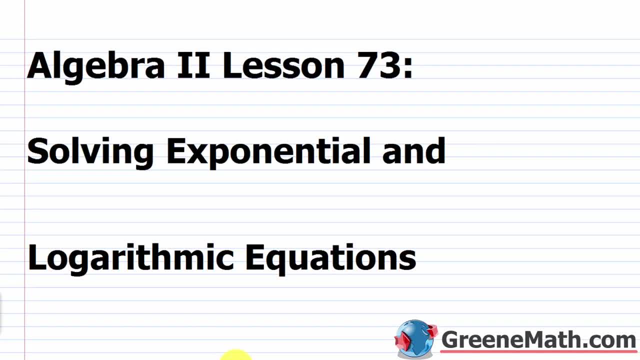 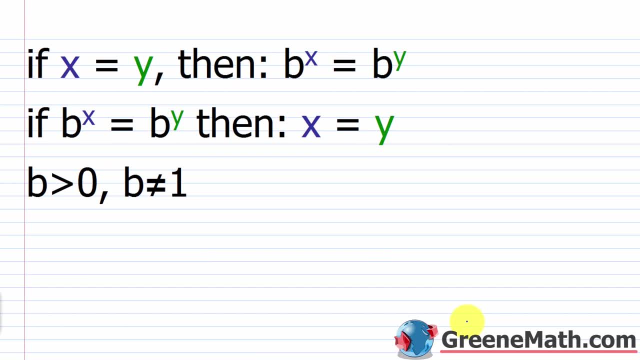 As a result. hello and welcome to Algebra 2, Lesson 73.. In this lesson, we're going to learn about solving exponential and logarithmic equations. So, although we've seen how to solve an exponential equation before, and also we've seen how to solve a logarithmic equation before, 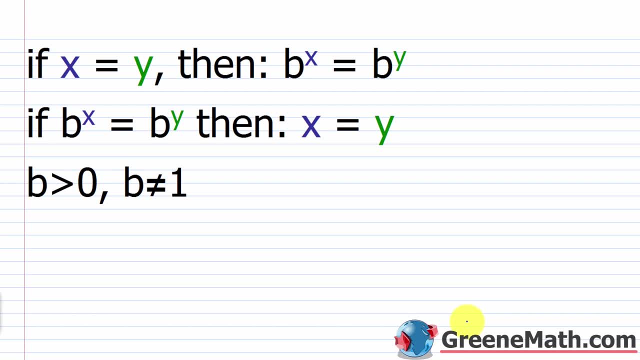 the problems we're going to deal with here are going to be significantly more difficult. So in order to get through them, we have to go through a few properties real fast. So this property here. you've already seen it when we solved exponential equations. 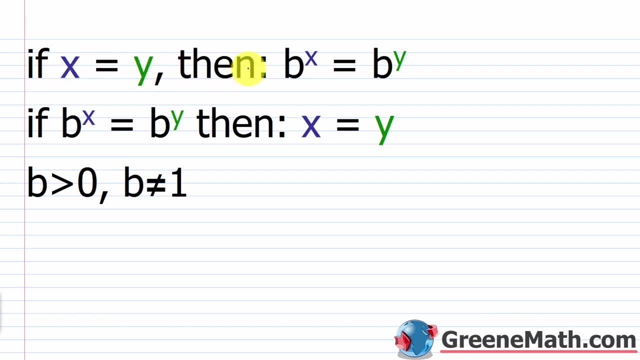 equations. We say: if x equals y, then b raised to the power of x is equal to b raised to the power of y. Or you could also say: if b raised to the power of x equals b raised to the power of y, then x is equal to y. Now the restrictions here say that b- your base has to be greater than zero. 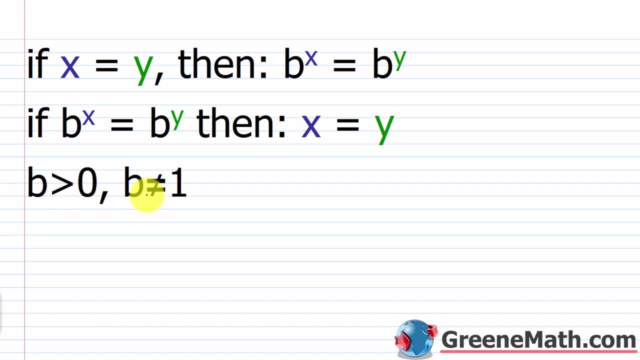 so it's got to be positive And also it's not allowed to be equal to one. So, given that you follow those restrictions, if you have something that sets up like this: b to the x equals b to the power of y, so in other words the base is the same, then you can set x equal to y and you 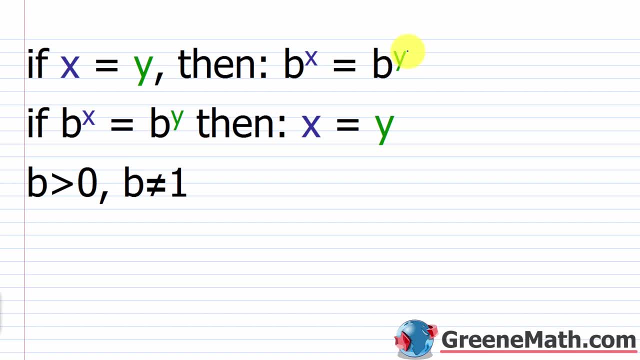 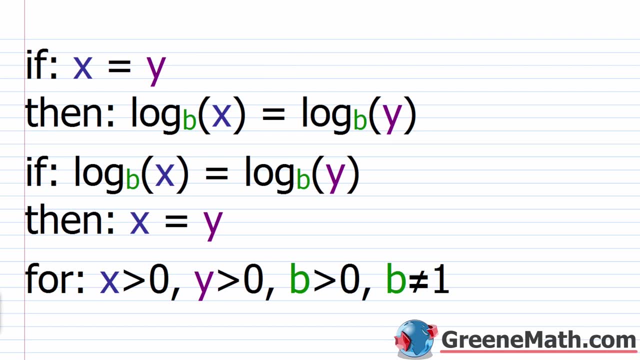 can solve. We've already experienced that before. We would make our bases the same, we would set the exponents equal to each other and we would solve and get our answer. Now let's talk about some other properties. If x equals y, then we can say that log base b of x is equal to log base b of 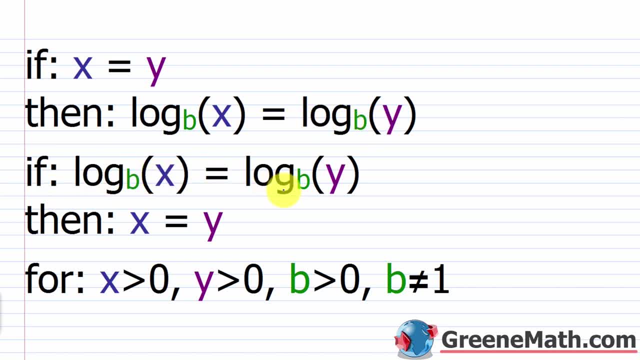 y. We could also say: if log base b of x equals log base b of y, then x is equal to y. Now you have more restrictions here. We say that this is for: x is greater than zero, y is greater than zero. 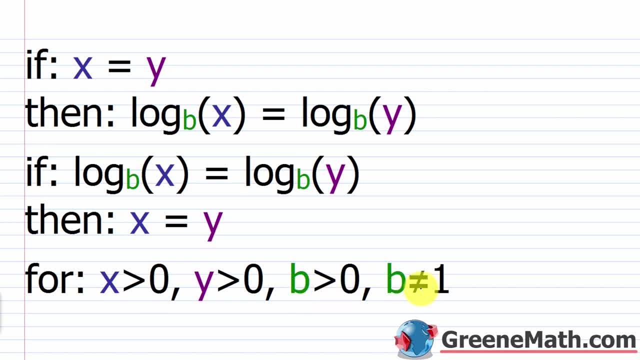 b is greater than zero and b is not allowed to be equal to one. So x and y here represent arguments in the logarithms. So here's x here, here's y here. Remember those have to be greater than zero. The base, here the b we say, has to be greater than zero and again, it's not allowed to. 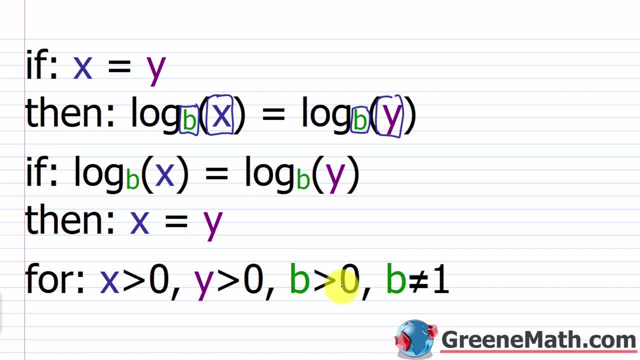 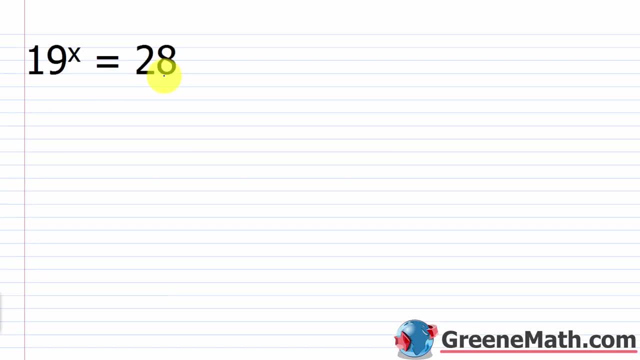 be equal to one. So we're going to use these properties. You might want to pause the video and just write them down. We're going to use them as we start to solve these equations. All right, so we're going to start off by just looking at some exponential equations, and the first guy. 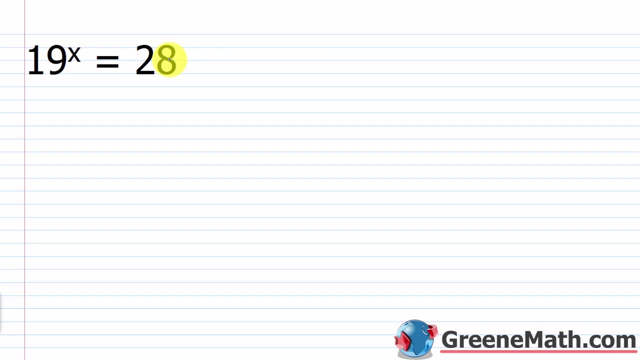 we're going to look at is 19 to the power of x equals 28.. Now, a few lessons ago, we looked at easier examples where we could just make the bases the same. we could set the exponents equal to each other and then we would solve. That's not going to work for us here, so we need to use a different. 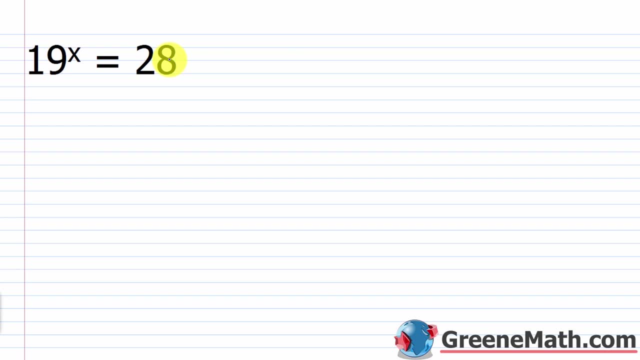 technique. In this case, we're going to take the log of each side and remember. we're going to take the log of each side and remember, if I have log base 10 of something, I don't need to write the base. 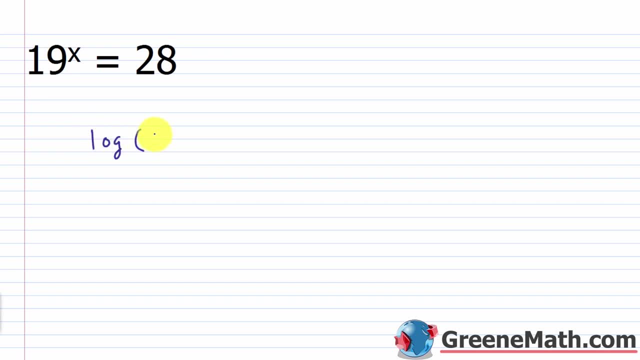 of 10, it's in plot. So I can say this is log of 19, raised to the power of x, this is equal to log of 28.. So I really didn't do anything special here. no magic tricks involved. I just took the log of. 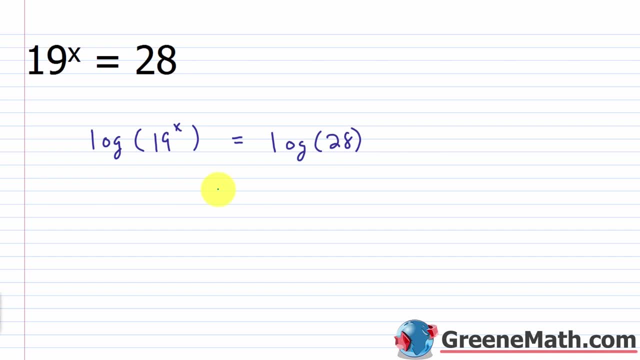 both sides. Now, what does this allow us to do? Remember that power rule for logarithms that we talked about a few lessons ago. That allows me to take this guy right here, the exponent, and bring it down here. So we're going to take this guy right here, the exponent, and bring it down here. So 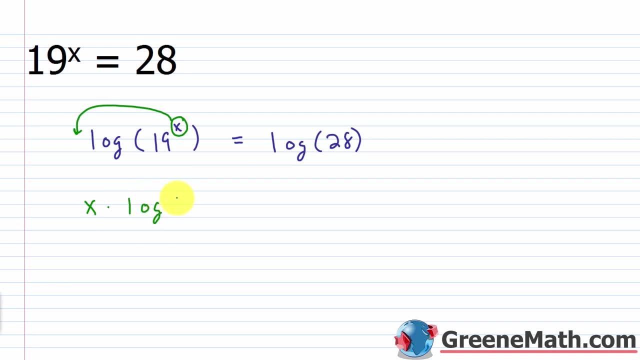 what's going to happen is I'm going to have x times log of 19, and this will be equal to log of 28.. Now, if I want to solve for x, I just want to isolate it. So what's multiplying x here? Well, 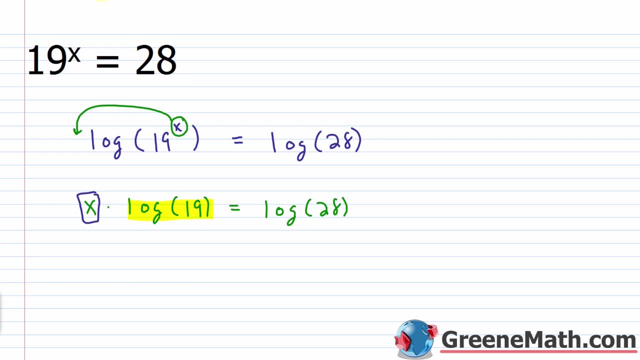 it's just log of 19.. So all I need to do is just divide both sides of the equation by log of 19, and I'm done So. it's very, very easy to solve a scenario like this. This guy right here will cancel with this guy and I'll have my answer. It's: x is equal to log of 28. 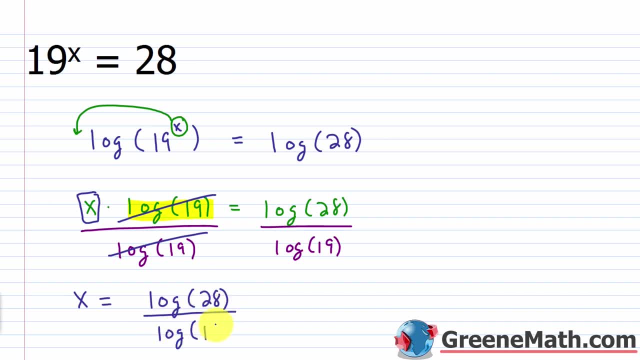 over log of 19.. Now, this is an exact value here. If you want an approximation, you can type that into a calculator and, depending on how accurate you want it to be, you can round or you can truncate. whatever you want to do, just make sure you use an approximation symbol versus an equal. 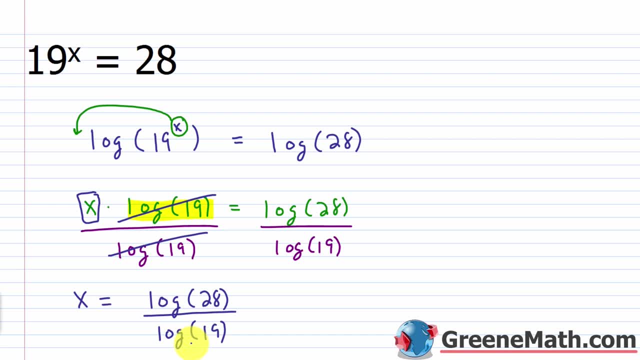 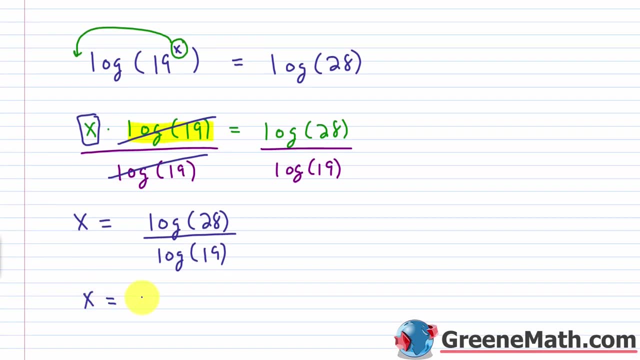 symbol to say hey, this is approximately this, versus saying it's exactly this. Another way we could write this: remember our change of base rule. So we could say: this is x is equal to log base 19 of 28.. Okay, so that's two different ways you can write this. I would probably stick to this. 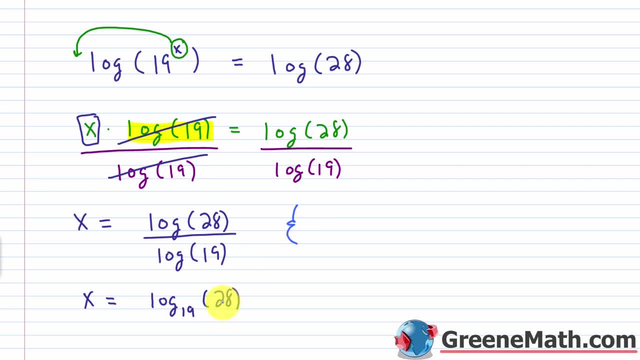 way right here. So in my solution set I will write the element as log of 28 over log of 19, and I keep it in that format because it's easier to type it into a calculator that way. So this is what I would report as my answer if I was on a test. but again, if you needed to give, 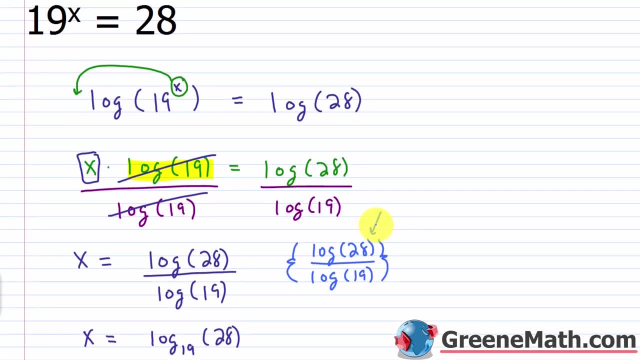 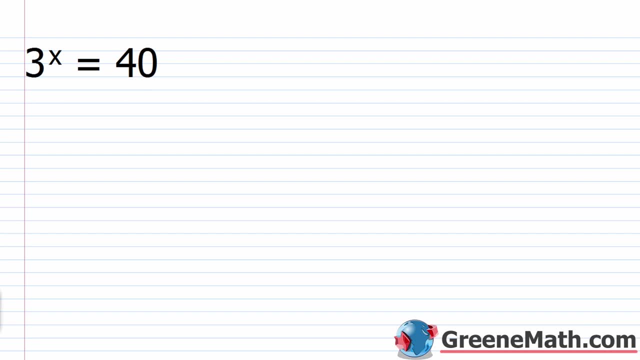 an approximation. you could just punch it into a calculator and give that. All right, let's take a look at another one. So we have 3 to the power of x equals 40. So we're going to do this the exact same way. Instead of using the common logarithm, let's kind of use the natural logarithm We can. 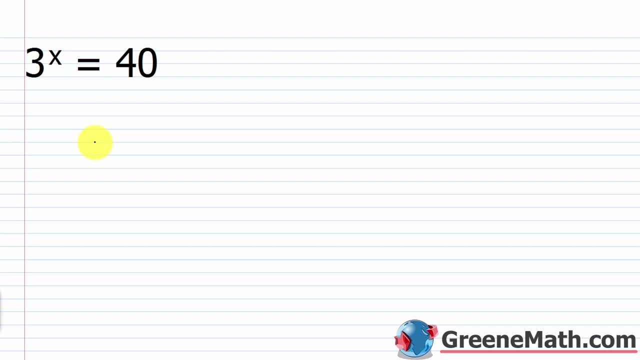 use either one. Both buttons are accessible on pretty much every calculator. So I'm going to say this is ln of 3 to the power of x is equal to ln of 40. And again, this is the exact same thing as if I would have done log of 3 to the power of x. 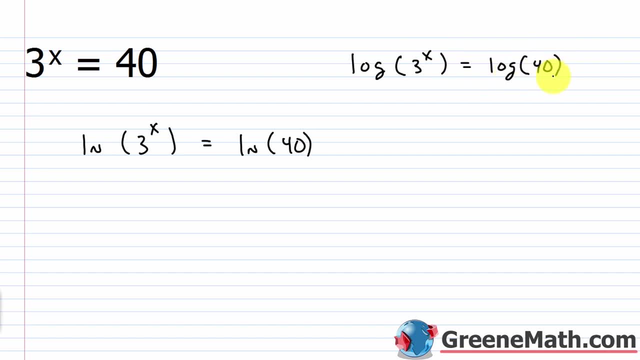 is equal to log of 40.. It's going to enable me to do the same thing. So this guy right here is going to come down, and so I'm going to have x times ln of 3 is equal to ln of 40.. 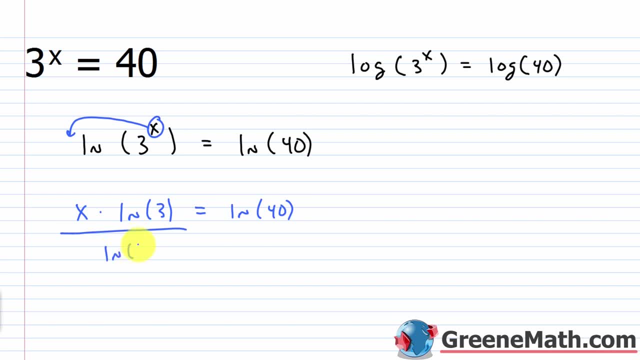 I divide both sides of the equation by ln of 3.. Again, that's what's multiplying x, And I'm going to have my answer. This cancels with this I'll have: x is equal to ln of 40 over ln of 3.. All right, so for my solution set, I'm going to put ln of 40 over ln of 3.. 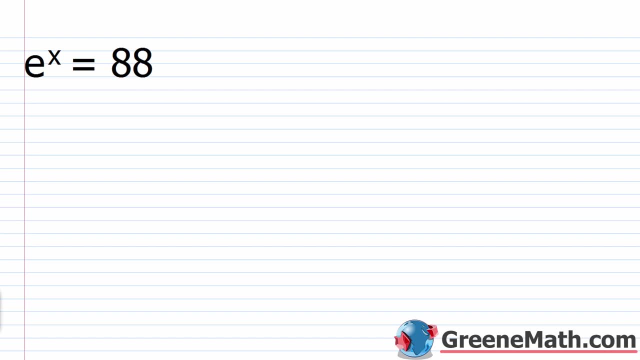 All right. so now we're going to look at one that involves the number e. So remember, this is a special universal constant, something like pi. So when e is involved, you always want to use the natural logarithm. You might say why? Well, if I take 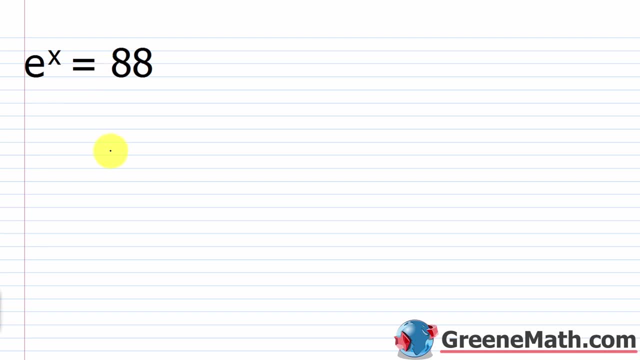 e to the power of x equals 88, and I say ln of e to the power of x equals ln of 88,. what's going to happen is this, right here, is going to cancel itself out and become 1.. So I'm going to have x equals ln of 88.. 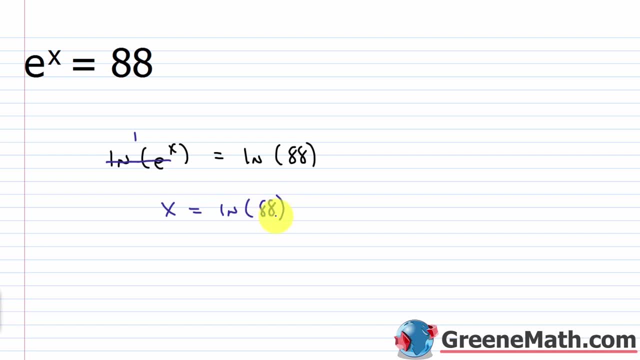 And I'm done. You might say: why in the world does ln of e equal 1?? Well, think about what ln actually means. Remember, ln is a log with a base of e. So really, what this was was, it was log. 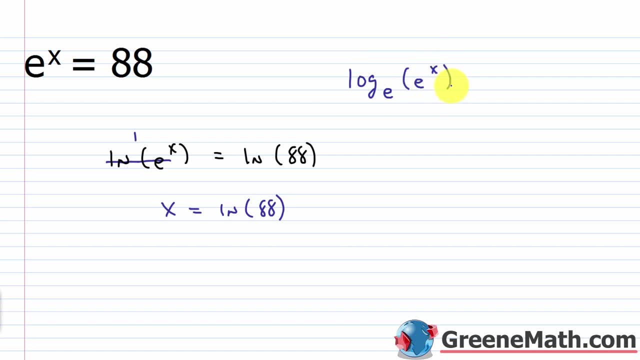 base e of e to the power of x. Now I can bring this guy down here, So really I'm saying this is x times log base e of e. So what is this part equal to? it's equal to one e to what power gives me e? one right e to the first power would give me back e. 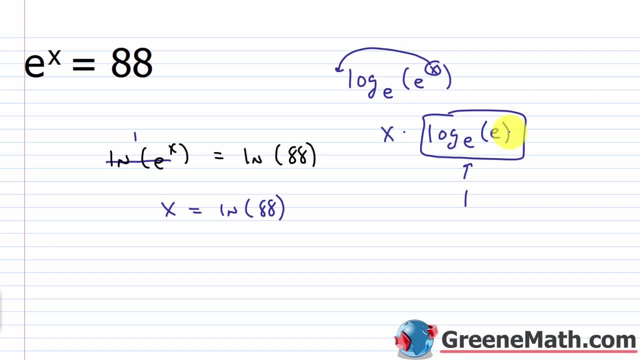 so when you have ln of e, that automatically equals one. so when i see something like that, i always want to use the natural logarithm. you could do this using the common logarithm if you want, but it's just going to be more work for you. so you want to stick to this technique? all right, so x. 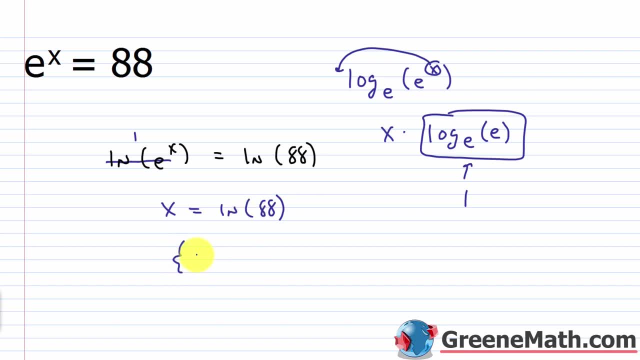 equals ln of 88, or in solution set notation, i'll just put ln of 88 like that. all right, let's take a look at another one. so we have e to the x equals 75. again, i'm going to use ln. so i'm going to use. 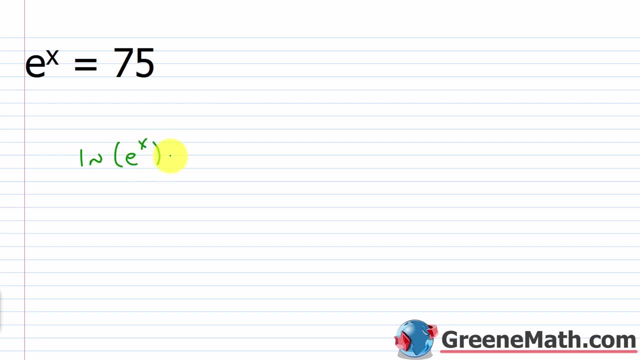 my natural log. so ln of e to the x is equal to ln of 75, and again this guy would come down here, so you'd have x times ln of e. we know that this guy equals 1. and we know that this guy equals 1. 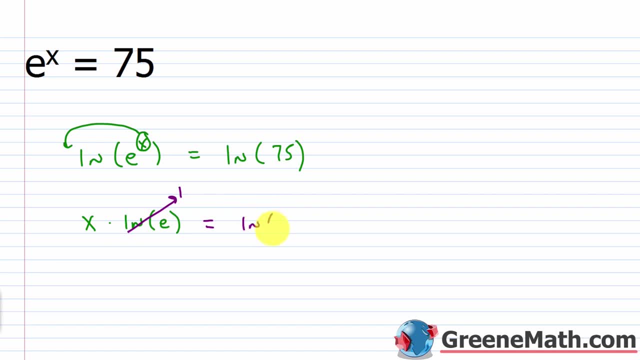 and we know that this guy equals 1, and we know that this guy equals 1: 1.. I just showed you that. So this would be equal to ln of 75. So there's your answer: You would have x equals ln of 75. So let's put this in solution set notation: ln of 75.. All right, 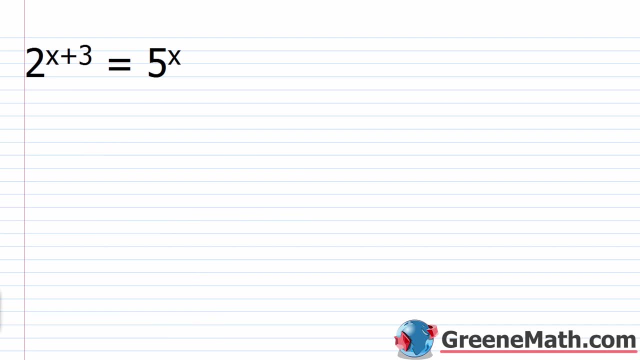 let's try a few that are a little bit more tedious, and then we'll move on and look at some logarithmic equations. So another thing you're going to see in this section is super hard. It's just a lot of things that you have to remember from all the things throughout the 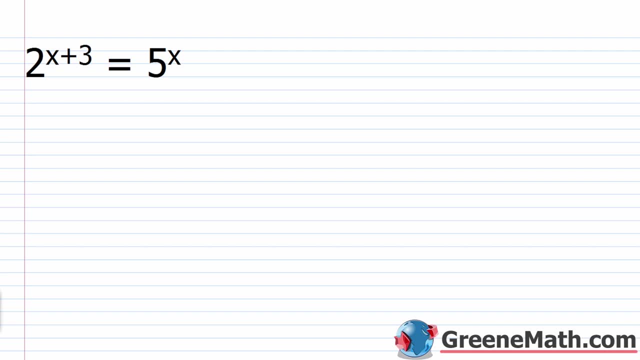 chapter where you're talking about exponentials and logarithms. So here we have: 2 raised to the power of x plus 3 equals 5 raised to the power of x. So I'm going to use my normal technique. I'm going to say this is log of 2 raised to the power of x plus 3 equals log of 5 to the power of. 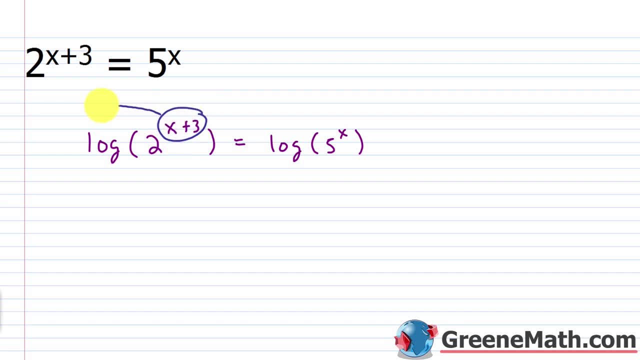 x. So what I'm going to do is I'm going to take these down, And so I'll have x plus 3, that quantity multiplied by ln of 75. So I'm going to say: this is log of 2, and this equals x multiplied by log of 5.. Now, in a lot of 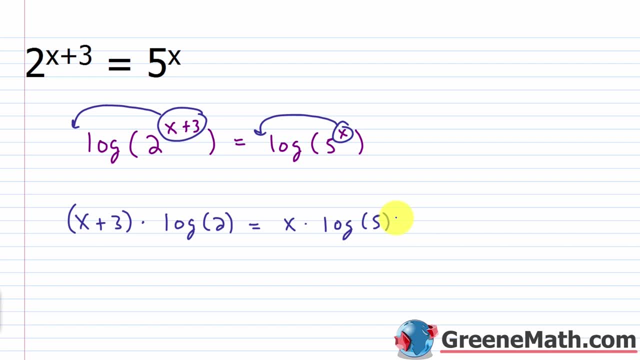 cases when people see this, they get stuck at this point. They're like: what do I do? How do I get x by itself? I've got x on this side. I've got x on this side, but it's wrapped in some. 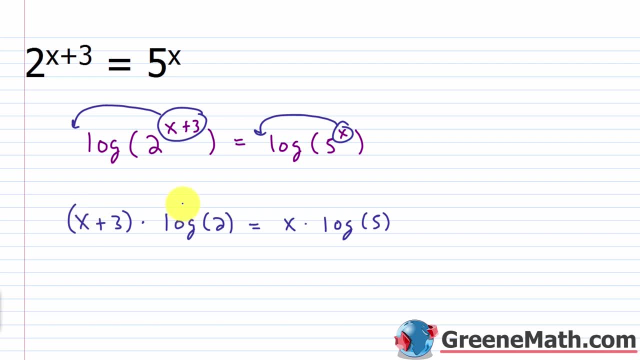 parentheses. Just realize that you're going to use your distributive property here. This is a number. If I had a number multiplied by the quantity x plus 3, I would just distribute it. So you're not going to use any different technique simply because you have a logarithm involved. It's just a number. So I'm. 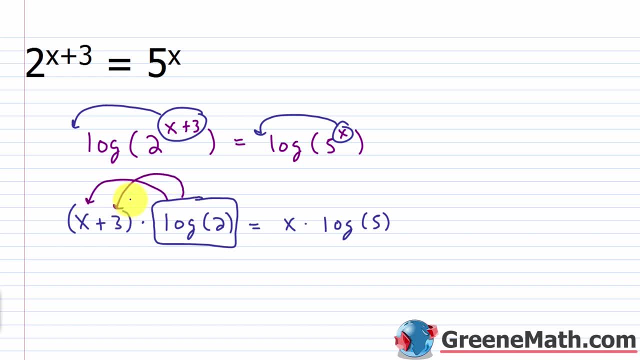 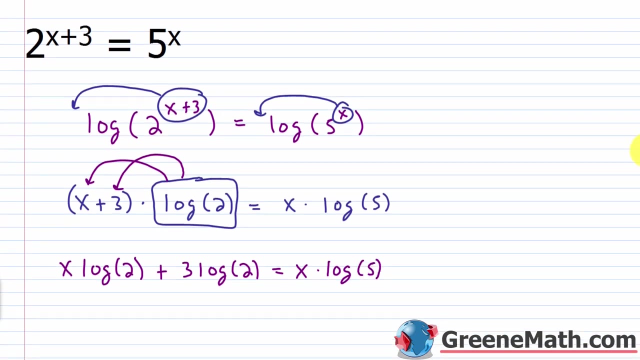 going to say: this times this plus this times this, So we'll have x times log of 2 plus 3 times log of 2.. And this is equal to x times log of 5.. Now, what do I want to do next? Well, what I want to. 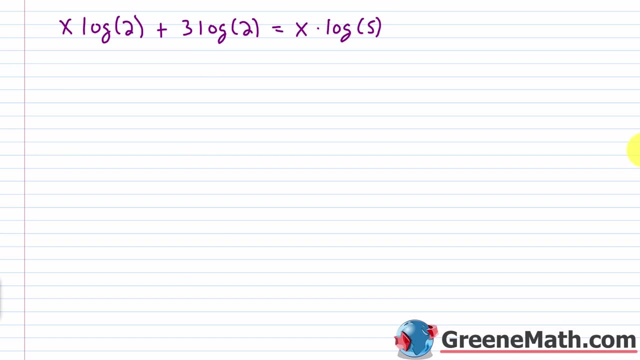 do is I want to get all the terms with x in it on one side of the equation, Everything else on the other. This is no different than what we've been doing forever. So let me subtract x times log of 5 from both sides of the equation. 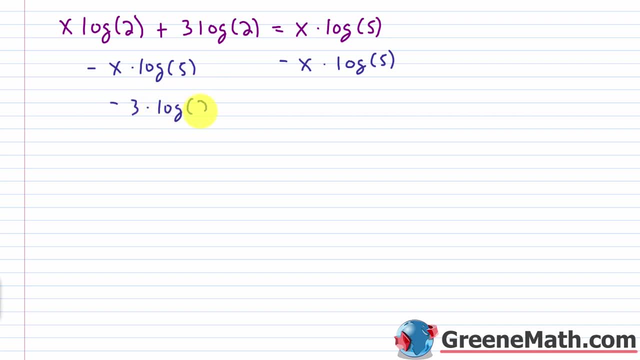 Let me also subtract 3 times log of 2 away from each side of the equation. So this would cancel with this and this would cancel with this. So what I'd be left with on the left is x times log of 2.. 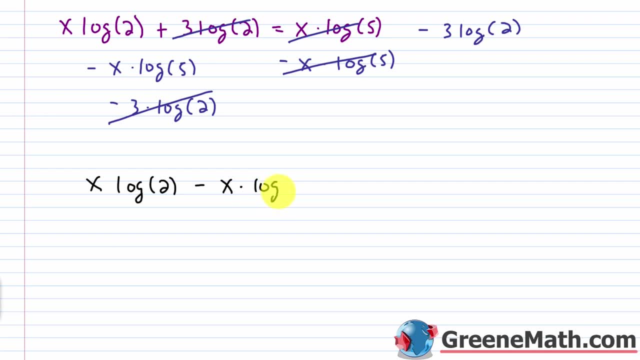 And then we'd have minus x times log of 5.. And this equals negative 3 times log of 2.. Now you might be saying: how in the world am I going to simplify this? You're going to factor, So remember, you have this here and this here. I could factor the x out. 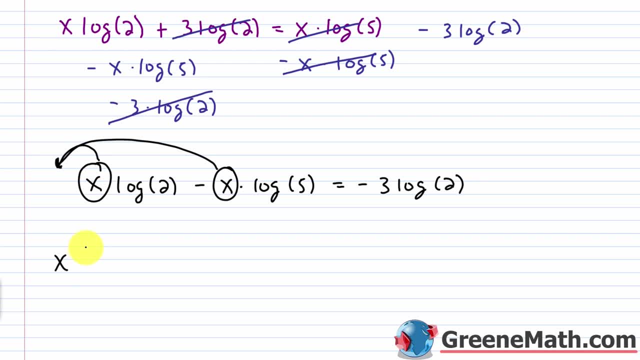 I could factor the x out and I would have x times inside of parentheses. you'd have log of 2 minus log of 3.. of 5, and then this is equal to negative 3 times log of 2. so at this point it's. 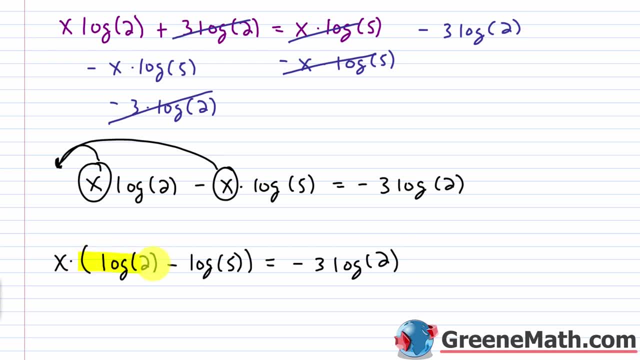 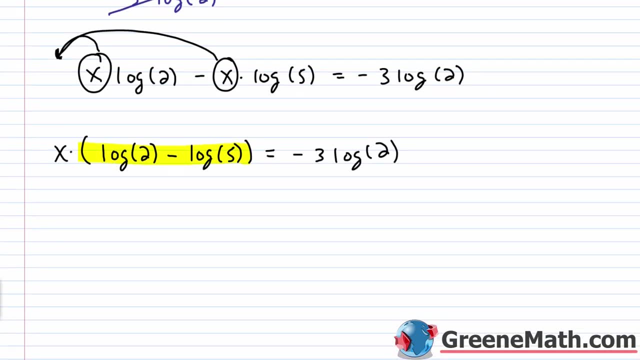 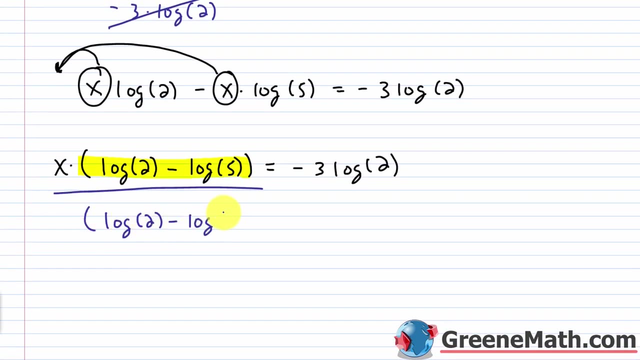 pretty easy to see that X is multiplying this guy right here, and so I would just divide both sides of the equation by that and I have my solution. let me kind of scooch this down a little bit, get some room. so I would divide both sides of the equation by this: log of 2 minus log of 5. so over log of 2 minus log of. 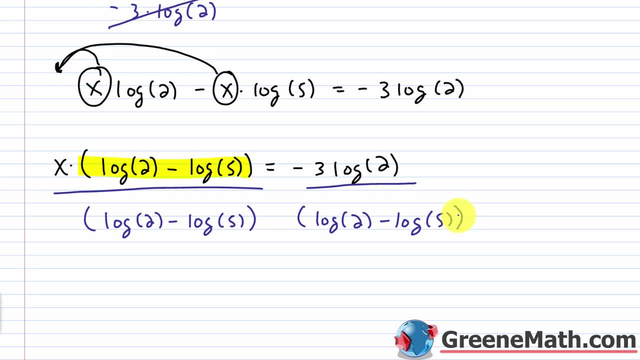 5, and this can get pretty tedious depending on what you're working with, but in the end it's no more difficult than solving anything else. you just got to take things one step at a time. so our answer here will be that X is equal to negative 3 times. log of 2. 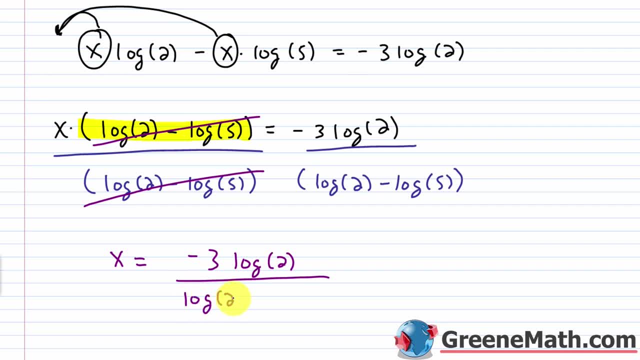 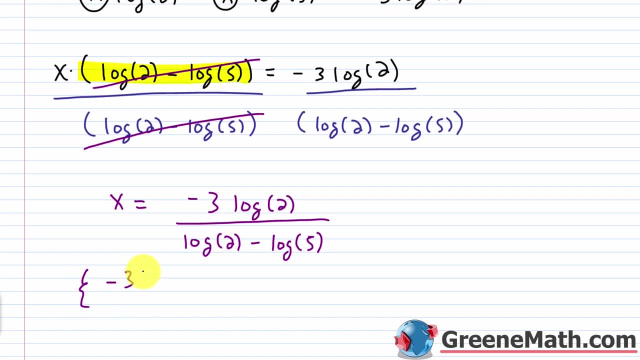 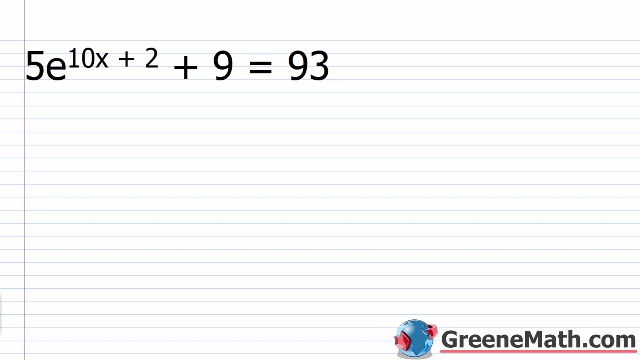 this is over. you have log of 2 minus log of 5 and in solution set notation I'll just put negative 3 times log of 2 over log of 2 minus log of 5. what about 5 times e? raised to the power of 10x plus 2 plus 9 equals 93. so in this scenario, 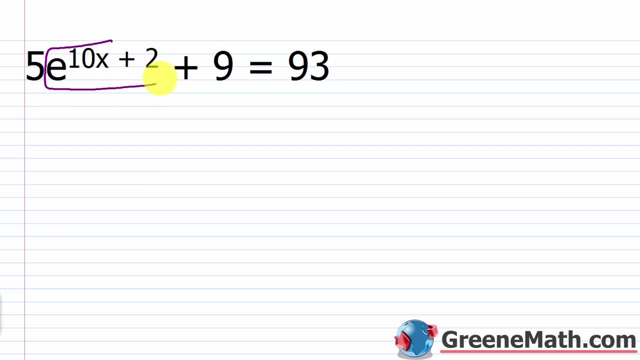 you want to kind of clean things up first. you want to try to isolate this part right here, and you want to try to isolate this part right here, and you So that I'll do in order to solve this equation right here. so what I'm gonna do in order to deal with that is just subtract 9 away from each side of 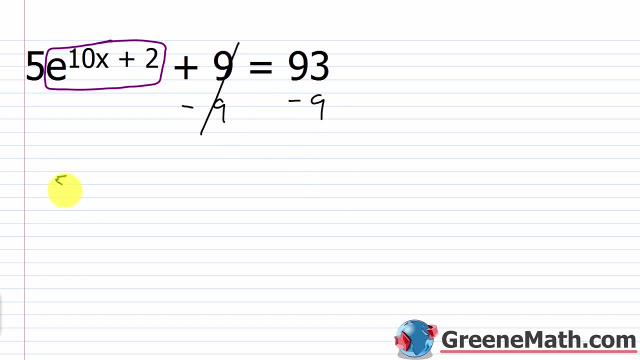 the equation first, so that I'll cancel. I'll have 5 times e raised to the power of 10x plus 2, and this is equal to 93 minus 9 is gonna give me 84. now again, I want this part by itself, so let me divide both sides of the equation by 5. 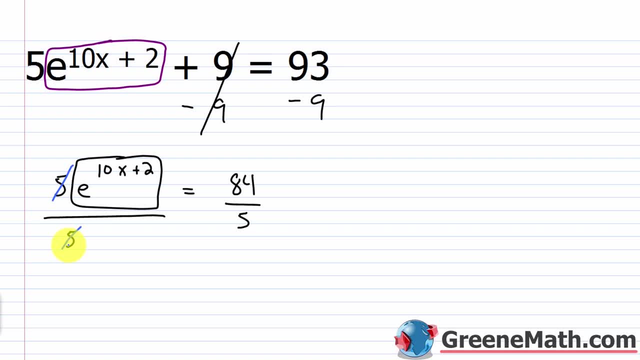 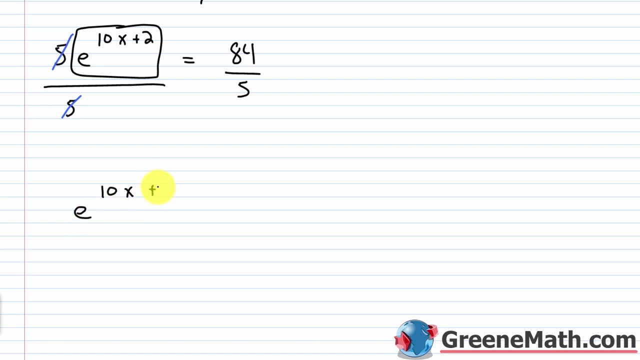 and so this will cancel with this, and now what I'm gonna have is something easy to work with. so if I do 2 times log of 2 vezes, log of 3 times the wrapped Rated R, to have e raised to the power of 10x plus 2. This is equal to 84 fifths. The reason I want this by 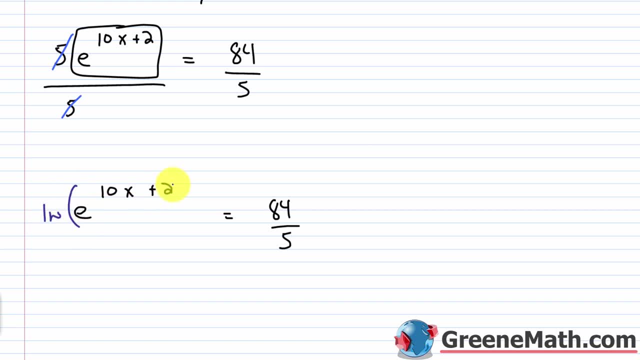 itself is because now I can just say: ln of this side equals ln of this side, right? So now I know that this e part in the ln will cancel right, They'll become 1.. So I'm just left with this part right here in the exponent, because that would have come down. So I would have: 10x plus 2 is equal to. 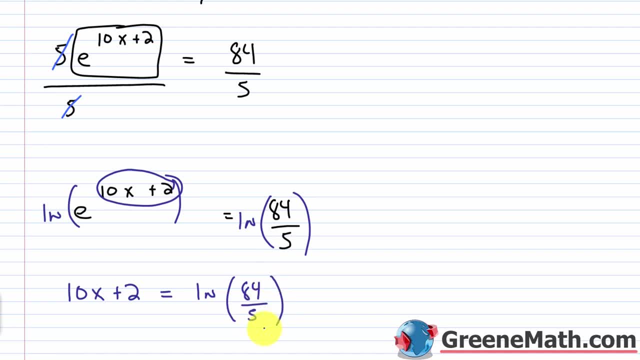 ln of 84 fifths. Now I've got some more work to do to solve for x, So let me kind of drag this up here. What I'll have is 10x plus 2 equals ln of 84 fifths. I will subtract 2 away from each side. 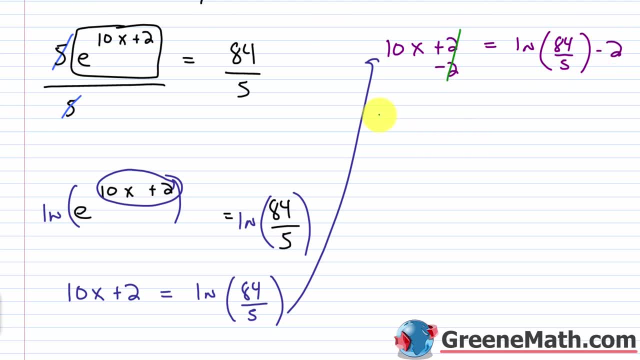 of the equation. So that's going to cancel. I'll have: 10x is equal to ln of 84 fifths minus 2.. I can divide both sides the equation by 10.. Over here, what I'm going to do is I'm just going to multiply the whole thing. 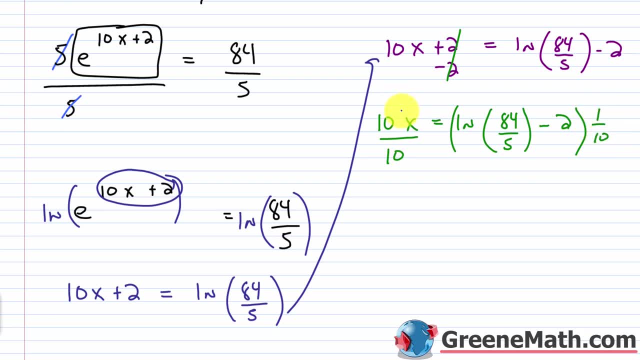 by 1 10th, just to make it a little easier on myself. So this will cancel. I'll have: x is equal to: you'll have ln of 84 fifths multiplied by 1 10th. then minus 2 times 1 10th, 2 times 1 10th. 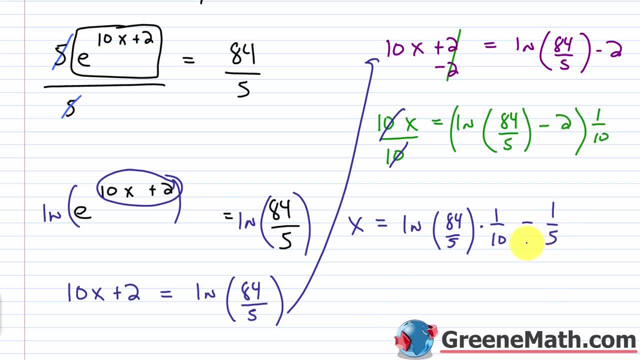 is 1 5th. So this would be my solution, So I could write it in solutions annotation. just say this: is 2 times 1 10th. 2 times 1 10th is 1 5th. 1 5th is 1 10th. 1 10th is 1 5th. 1 5th is 1 5th. So again, 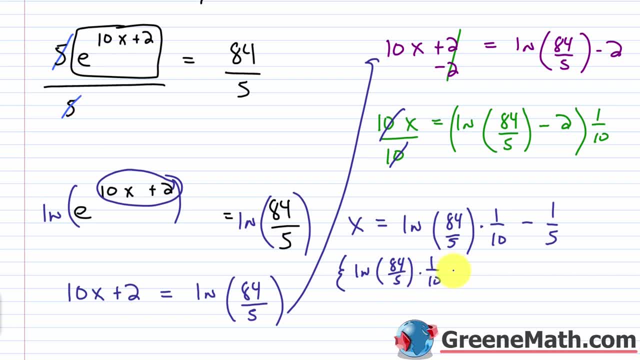 I might just go ahead and subtract 1 times the 1,, 2,, 4,, 3,, 4,, 5,, 6,, 7,, 8,, 9,, 10,, 11,, 12,, 13,, 14,, 15,, 16,, 17,. 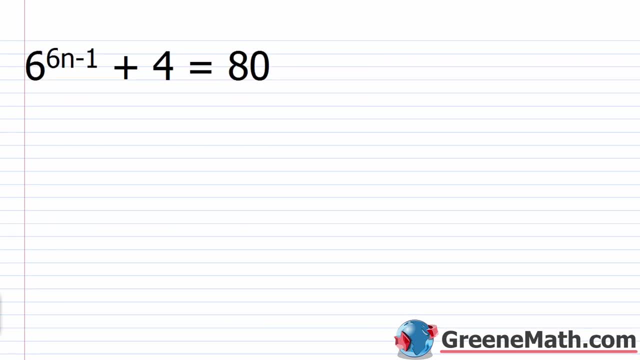 fifth, and again that's your answer. Let's take a look at one more of these and then we'll kind of move on and look at some logarithmic equations. So we have 6 raised to the power of 6n, minus 1 plus 4 equals 80. So I want to kind of clean it up. I want this by itself, So let me subtract 4. 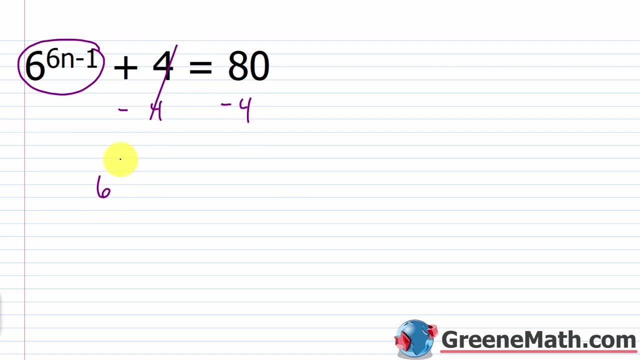 away from each side of the equation. to start, I'll have: 6 raised to the power of 6n minus 1 is equal to 76.. I'm going to take the log of both sides, So log of 6 raised to the power of 6n minus. 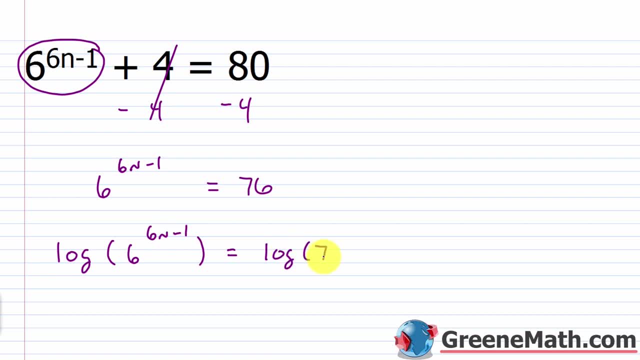 1 is equal to log of 76. So what this is going to again allow me to do is bring this down. So I'll have 6n minus 1 multiplied by log of 6 is equal to log of 76.. Scroll down and get a little bit of room going. So at this point, 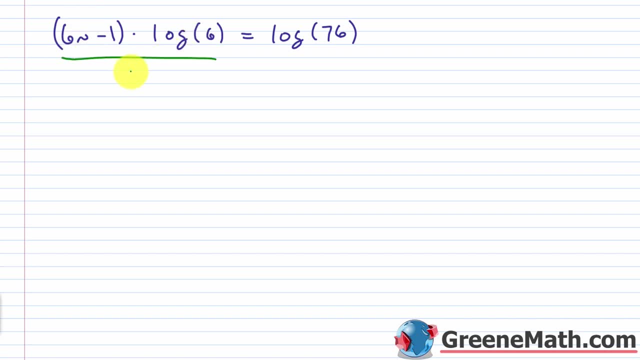 I can either use the distributive property or I can outright just divide by log of 6. So this would cancel, So I'd be left with 6n minus 1 is equal to log of 76 over log of 6.. 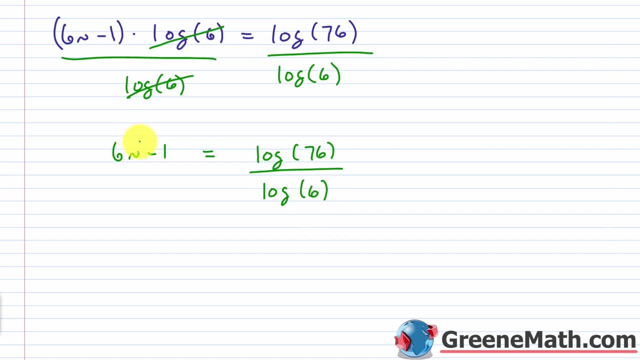 Okay, so what do we do now? We want this part by itself, right? We want the n by itself. So I need to add 1 to both sides. So that'll cancel. So we'll have 6n is equal to log of 76 over log of 6,. 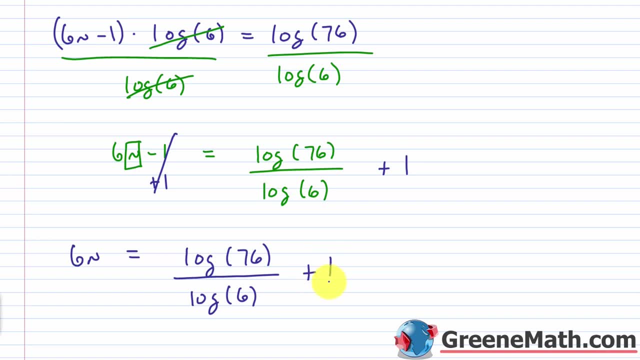 and then plus 1.. So the last thing I need to do is divide both sides of the equation by 6.. Again, if I'm going to do that, I'm just going to multiply this guy by 1 sixth, and that will allow. 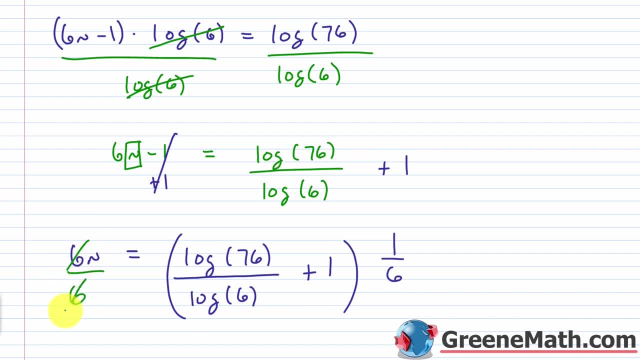 me to get n by itself. All right, let's scroll down and get a little bit more room going. So I'm going to divide both sides of the equation by 6.. And I'm going to divide both sides of the equation by 6.. And I'm going to divide both sides of the equation by 6.. And I'm going to divide both. 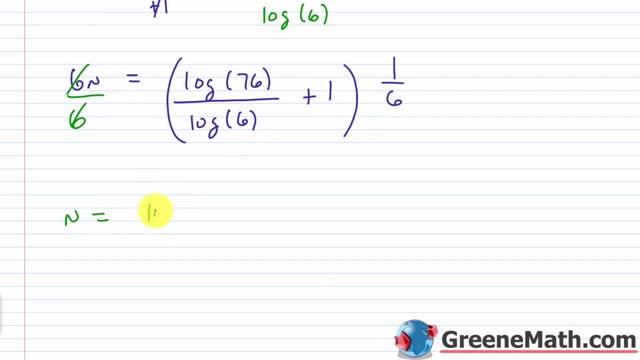 So we'll say n is equal to. we will have log of 76 over log of 6, then times 1 sixth, or you can put divided by 6, it doesn't really matter. Then plus 1 sixth times 1 would just be 1 sixth, So plus 1. 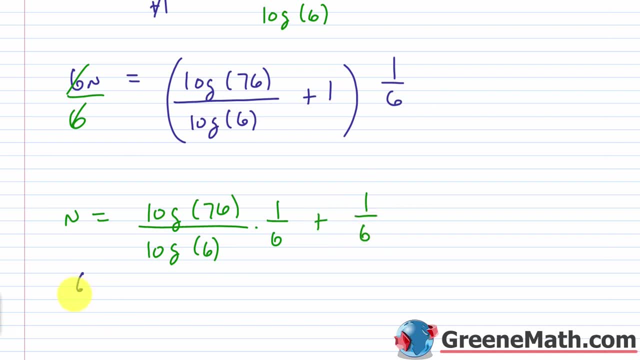 sixth over here. So in solution set notation I'm just going to say log of 76 over log of 6, multiplied by 1 sixth, Then plus 1 sixth, and that's going to be your solution. All right, now let's take a look at some. 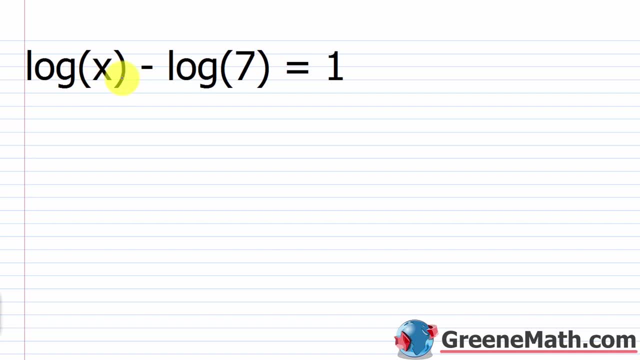 logarithmic equations. So let's say we saw log of x minus log of 7 equals 1.. So what would we do? We would use our properties of logarithms to rewrite the left side as one single logarithm. So if I have subtraction here, remember I'm allowed to condense. this Subtraction is related. 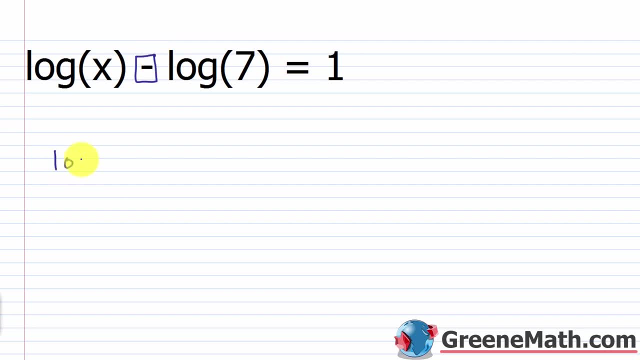 to division when we think about logarithms. So this would be log of the first guy I'm going to write here will go on the numerator and then you have your subtraction. so this is divided by This guy right here. the second guy is going to go on your denominator and then, of course, this is equal to 1.. So now that we 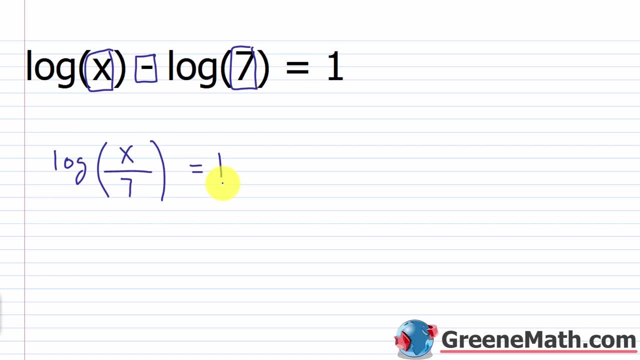 have this set up in this manner. how can we solve this? Well, we can write this using exponential form, and then it's easy to solve. So remember, this is log base. 10 of x over 7 equals 1.. So, in other words, this is 10 to the. 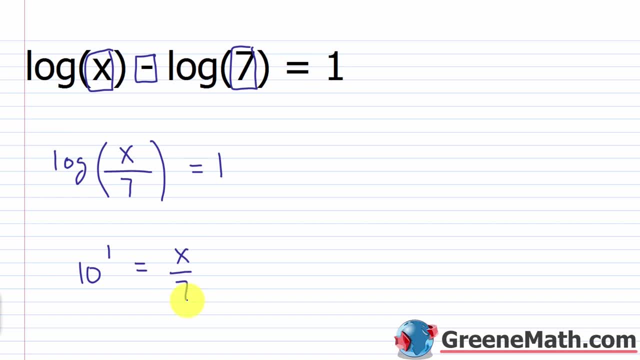 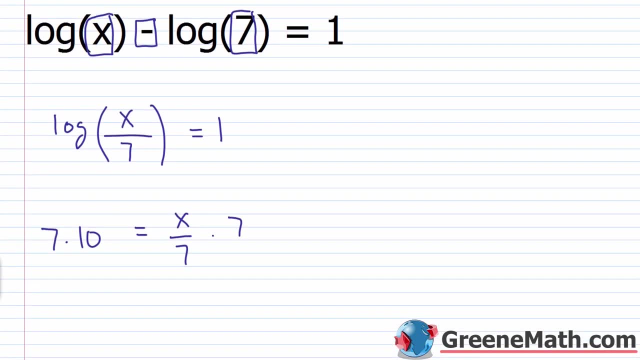 first power, 10 to the first power, is equal to x over 7.. Pretty simple equation to solve. I would simply multiply both sides of the equation by 7, and what's going to happen is I get: 70 is equal to x, or my solution. 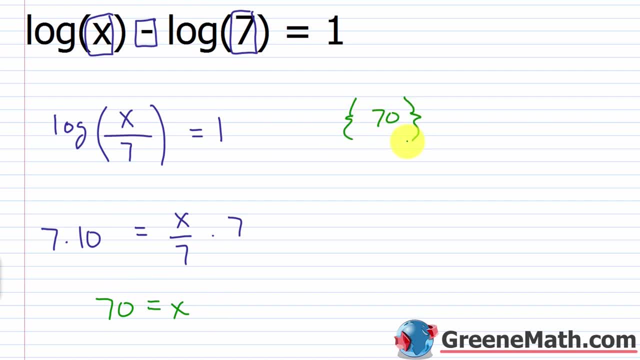 here is just 7.. Now if you plug that back in you can easily see that makes sense. If I had a 70 here, 70 over 7 is 10, so I'd have log base. 10 of 10 is equal to 1. That's true. 10 to the first power. 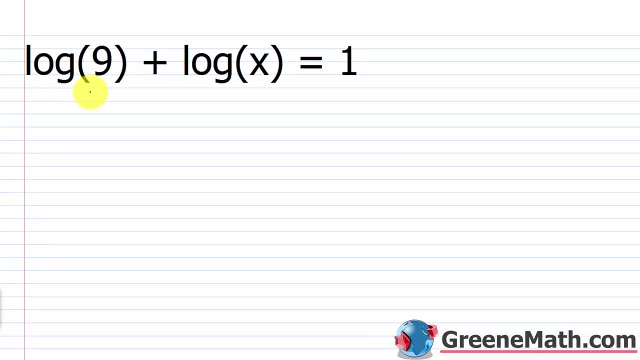 does give me 10.. So let's take a look at another one. So we have log of 9 plus log of x equals 1.. So again, what I want to do is use my properties of logarithms to condense this to 1 log on the left side of the equation. So, because this is addition, I'm 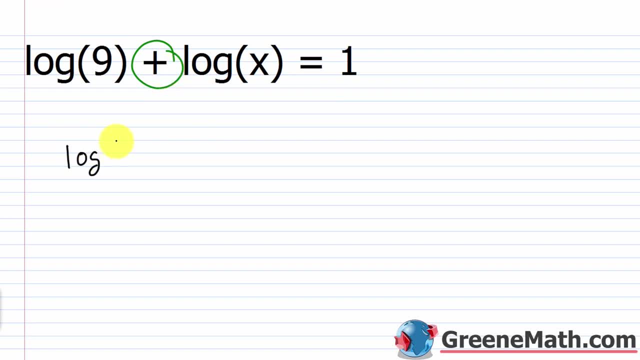 going to condense using multiplication. So this is going to be log of this guy times this guy. So 9 times x is 9x. This equals 1.. And again, all I want to do at this point is just use exponential form. So I know the base here is 9x and I want to use 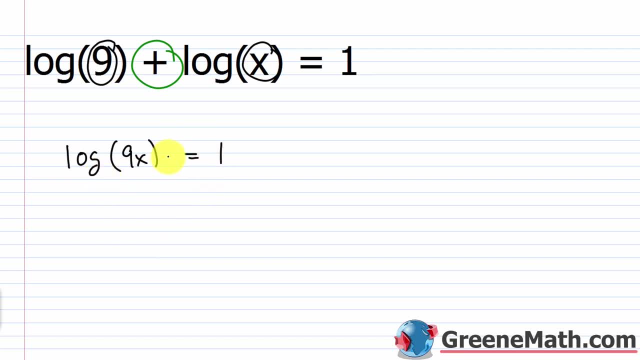 M. You're required to cancel between first power and third power, So that's everything you need here. Let's use unbelief. What's that mean if this is entails 10: 1.. of this guy right here, which is negative 4x divided by this guy right here, which is 5, this 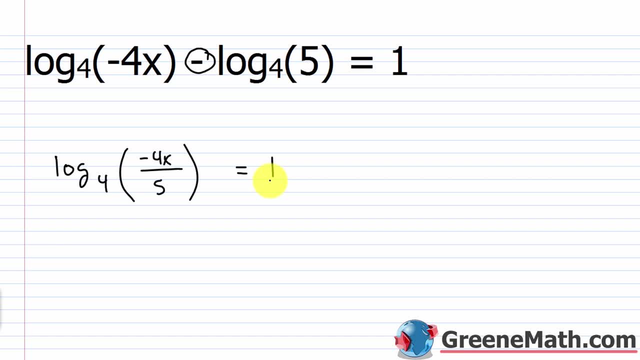 is equal to 1.. So I want to convert this into exponential form. so it's: 4 to the first power is equal to negative 4x over 5.. So 4 to the first power equals negative 4x over 5.. If I wanted to, 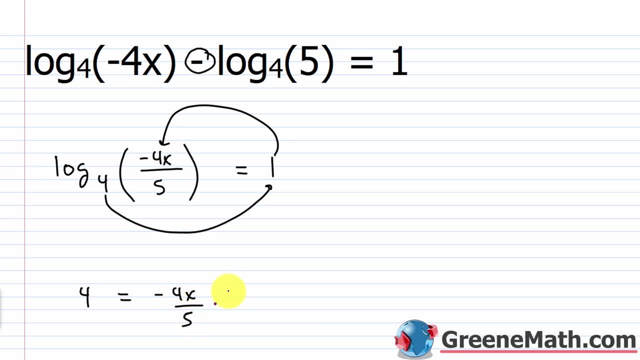 solve this. I'd multiply both sides by the reciprocal of negative 4 fifths, which is negative 5 fourths. so this part would cancel and I would have x is equal to 4s would cancel, so just negative 5.. Now you got to be careful here. remember your argument, for the logarithm has to be greater. 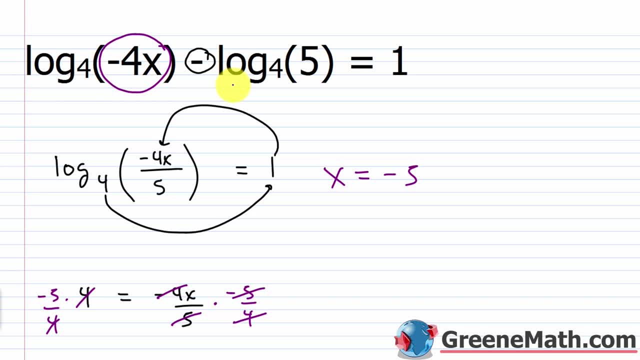 than 0. So if you end up with some answer that makes it negative or 0, you got to reject it, okay, so that's what you're looking for. If I plugged in a negative 5 there, negative 4 times negative 5 would be 20.. 20 is a positive. so I'm going to plug in a negative 5 there and I'm going to plug in a 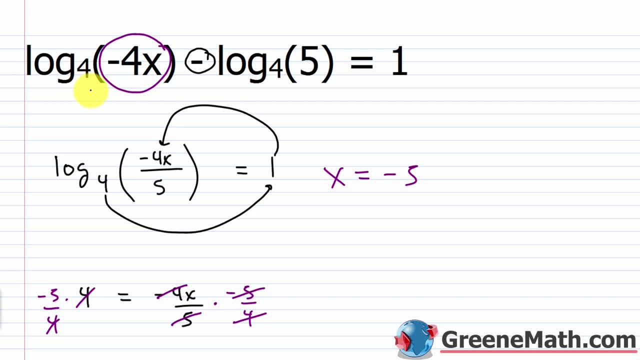 positive number. so you're good to go. This would be: log base 4 of 20 minus log base 4 of 5 equals 1.. What would that work out to be if we wanted to check it? So that would be log base 4 of 20 over. 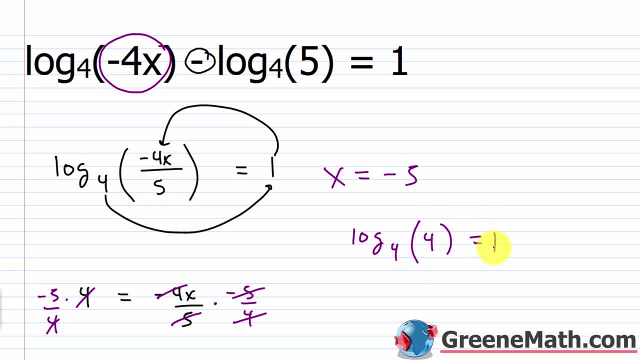 5 is 4, so log base 4 of 4 equals 1, so that does check itself out. and then in solution set notation I'll just put negative 5 inside of set braces. All right, what about log base 2 of 5 minus log. 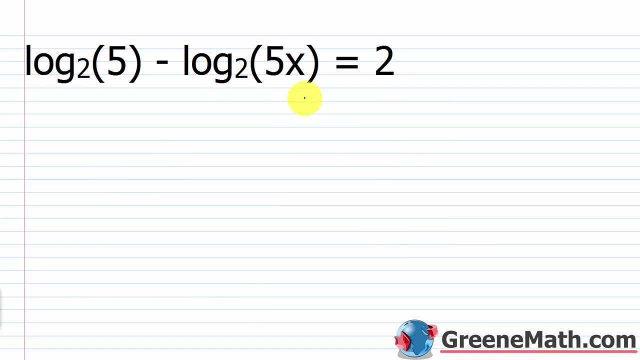 base 2 of 5x equals 2.. Again, I'm going to condense this. I'm going to put negative 5 inside of set braces, All right, so this is going to be log base 2 of positive root of positive 2.. So I'm going to 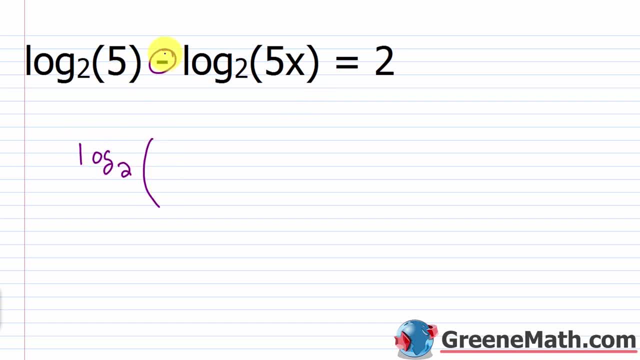 plug in a negative 5 divided by negative 3, which is negative 1 plus 2x plus 1.. So I'm going to plug it in this left side. This will be log base 2 of I have subtraction, so that's going to mean division. 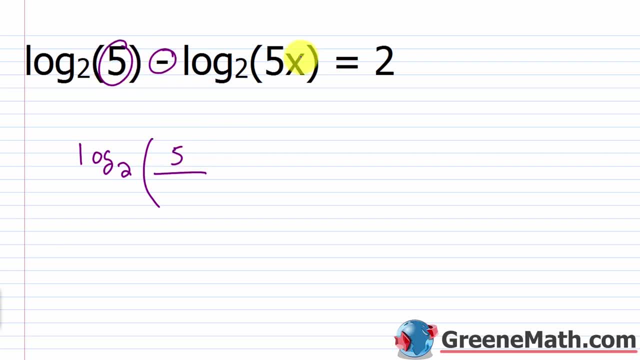 So 5- this guy right here- divided by 5x- that guy right there- This will be equal to 2.. So 2 to the 2nd power is going to give me 5 over 5x. 2 to the 2nd power equals 5 over 5x. Okay, so let's go ahead. 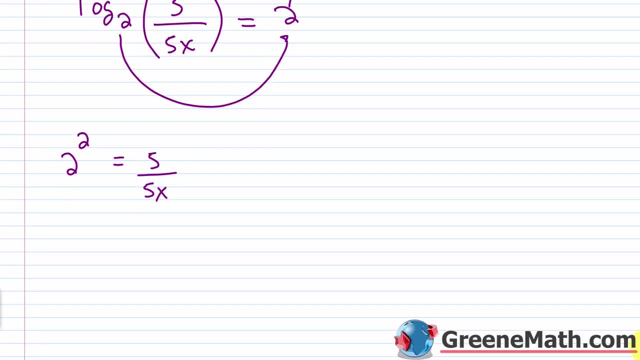 and solve this guy. We know that 2 is a positive, We know that 2 is a negative, We know that 2 is a square, would be 4.. So we would get: 4 is equal to 5 over 5x, So I know these 5s would cancel. 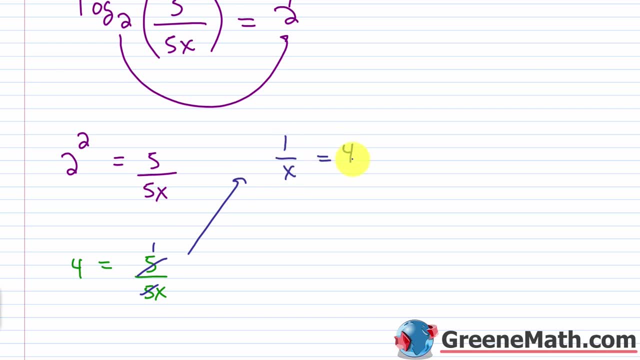 and so this would turn into: 1 over x is equal to 4.. If I wanted to solve this, an easy way to think about this is that this is x to the power of negative. 1 equals 4.. I could raise both sides. 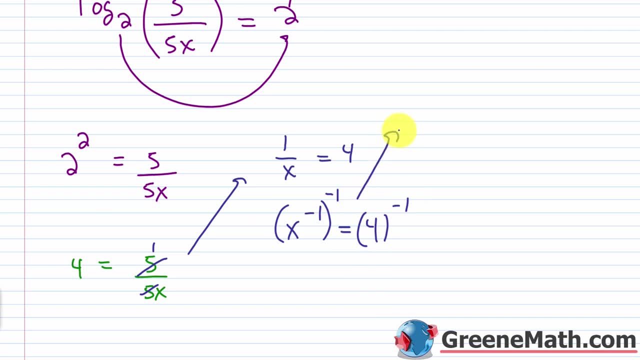 of the equation to the power of negative 1, and I'd have my solution. So negative 1 times negative 1 will be 1, so this would be x. now This is equal to 4 raised to the power of negative 1. 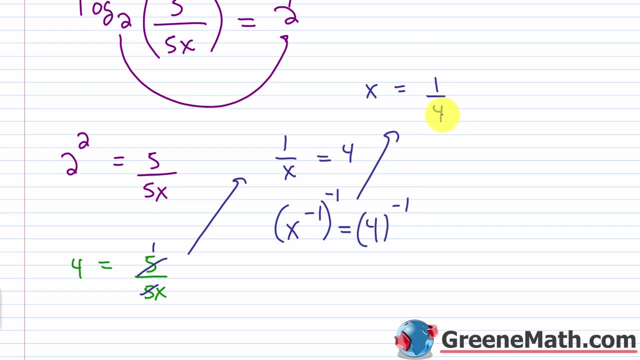 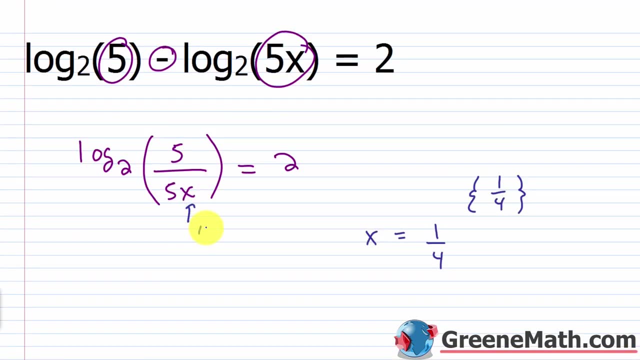 is 1 4th. So x here would equal 1 4th. And if you wanted to check, think about plugging in a 1 4th there. What would that do? You'd have 5 times 1 4th, which would be 5 4ths. You'd have log base. 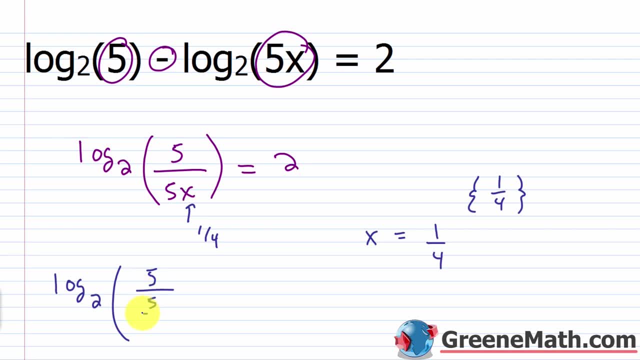 2 of 5 over 5 4ths. So 5 over 5 4ths. you can think about that as 5 over 5 4ths. So 5 over 5 4ths. you can think about that as 5 over 5 4ths. 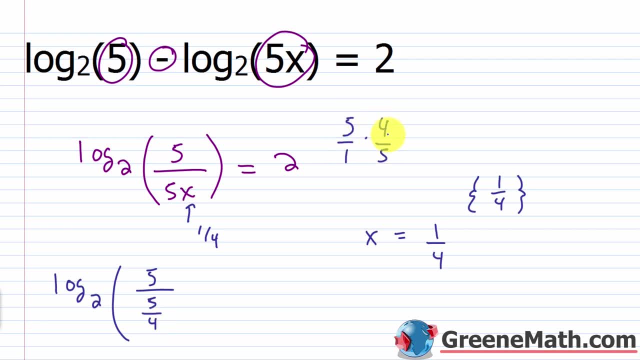 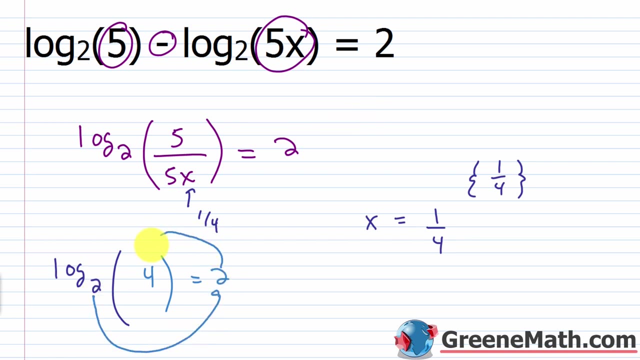 5 over 1 times 4 over 5.. The 5s would cancel and you'd be left with 4.. So really, this is 4 right here. So log base 2 of 4 is equal to 2.. Is that true? Well, is 2 squared equal to 4?? Yes, it is. 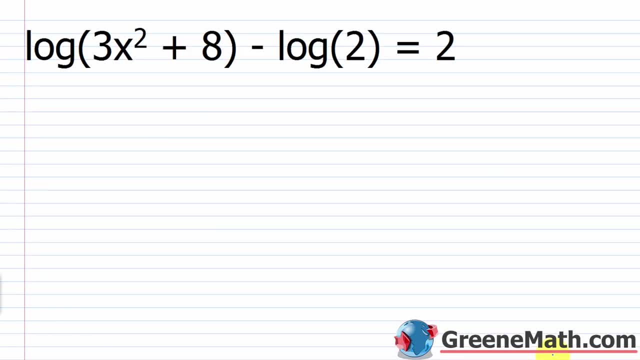 So this does check out. Let's take a look at log of 3x squared plus 8, minus log of 2 is equal to 2.. So again, I'm going to condense this Because I have subtraction involved there. So I'll have log of it'll be 3x squared plus 8.. 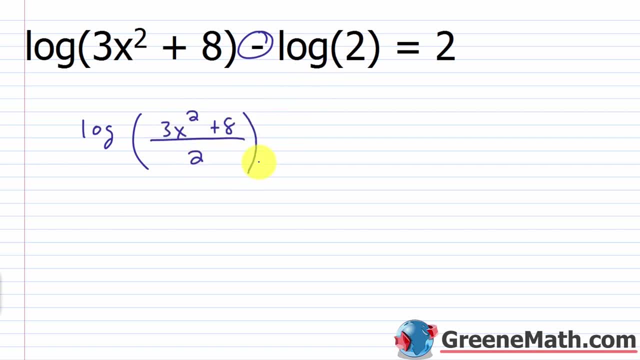 That'll be in the numerator over 2, which will be in the denominator. This is equal to 2.. So in exponential form I would have 10 raised to the power of 2, or you could say 100, is equal to 3x squared plus 8 over 2.. Now to get rid of the denominator there. 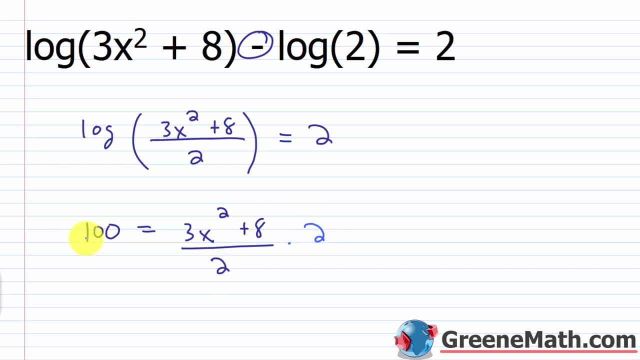 I can multiply both sides by 2.. So if I multiply this side by 2 and this side by 2, I would have 200 is equal to 3x squared plus 8.. I would subtract 8 away from each side of the equation So that would give me 192 is equal to. 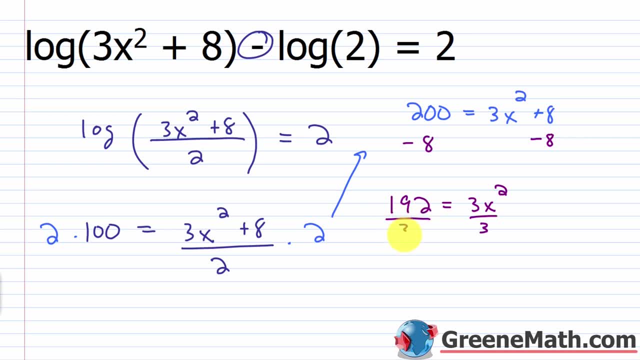 3x squared, I would divide both sides of the equation by 3.. Let's kind of erase over here real quick. So 192 divided by 3 would give me 64.. So I would have this canceling with this x squared. 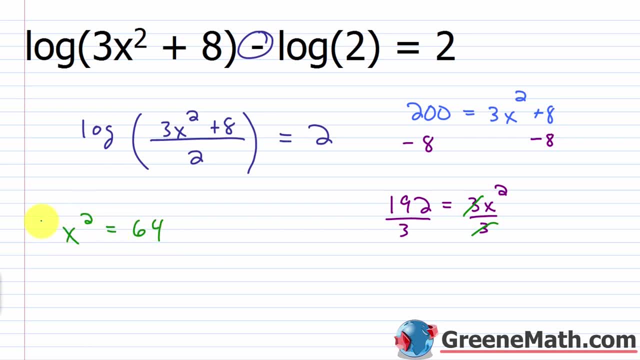 Now x squared is equal to 64.. Now I'm going to take the square root of each side and you'll have: x is equal to plus or minus. the square root of 64 is 8.. Now you do want to check to make sure that nothing you plug in here is going to make this guy. 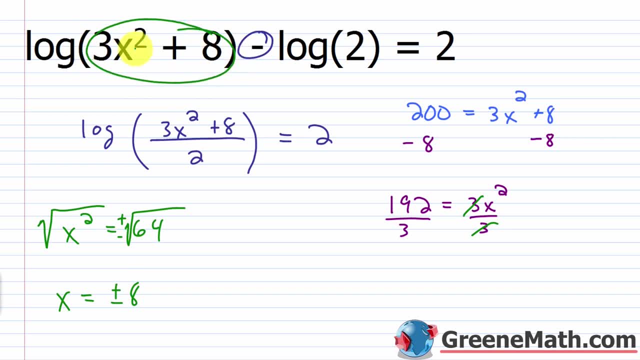 zero or negative. Remember, the argument's got to be positive. This one right here. you're not going to change, It's set as 2.. You just have to worry about that one. So if I plugged in a negative 8 there, it would be squared right. 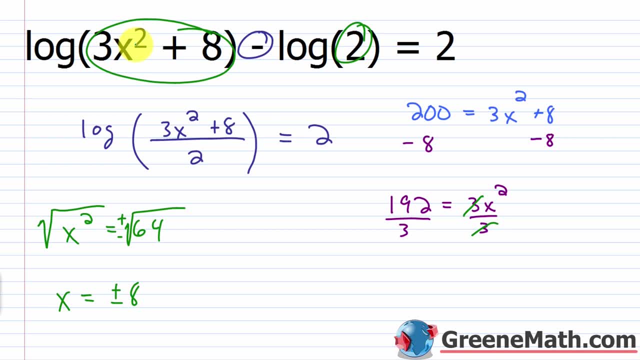 if I square that, it'd be 64.. 64 times 3 would give me 192.. 192 plus 8 would give me 200. So essentially you would have 200 divided by 2, which would be 100.. So that does work itself out. 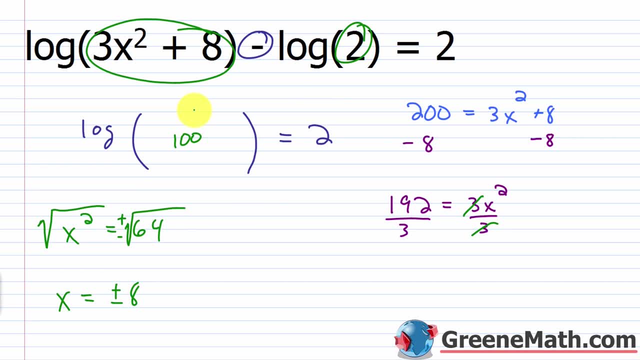 In other words, you're saying 10 to the second power gives you 100. So that works. Whether I plugged in an 8 there or a negative 8, I would not end up with a negative argument because of the squaring operation there. So I'm good to go right. Either way, I wouldn't end up with 100. 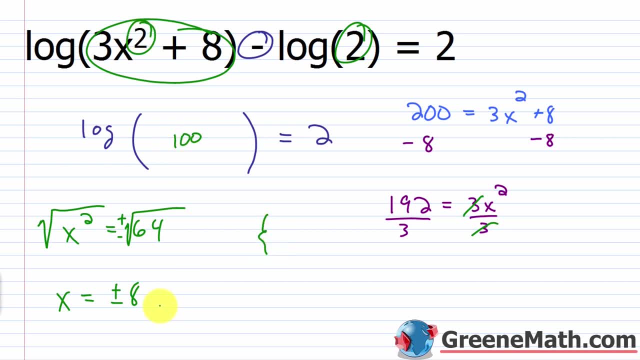 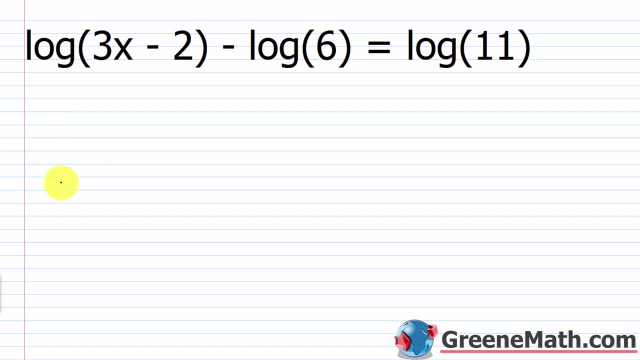 right there. So this answer here we'll go ahead and put in set braces. We'll put plus or minus 8.. All right, let's take a look at one more problem. So we have log of 3x minus 2, minus log of 6. 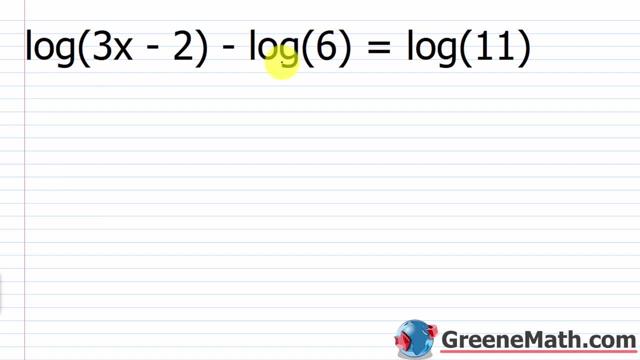 equals log of 11.. So I'm going to condense the left side. So we're going to say this is log of 3x minus 2.. I've got subtraction, so it's divided by that 6 there. This equals log of 11.. 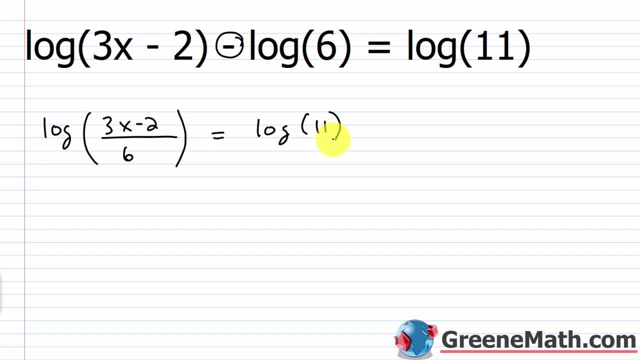 Now I could go through and solve this a different way, but the easiest way to solve this is to realize I have the same base here. So we already talked about in the properties if you had log, in this case it's base 10, so log base 10 of something equals log base 10 of. 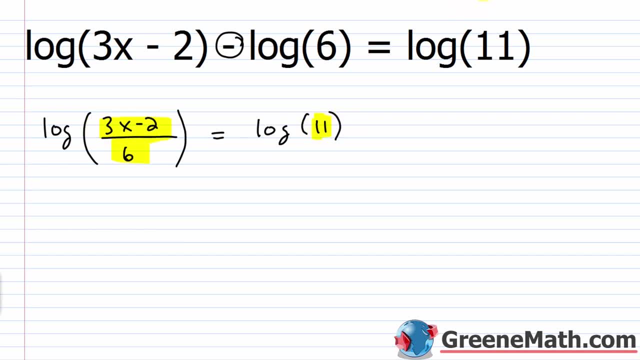 something else. the two arguments here are going to be equal to each other, So I can just set 3x minus 2 over 6, equal to 11, and I can solve. So let's start by multiplying both sides of the equation by 6.. 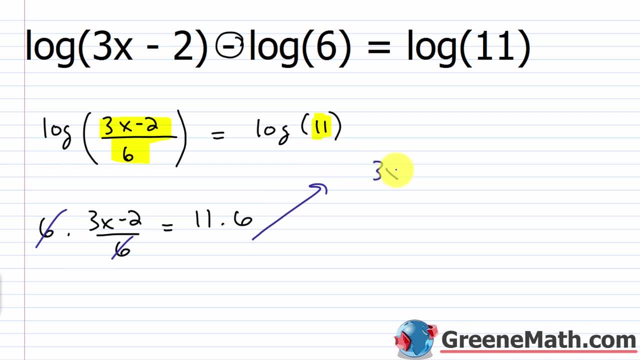 This will cancel. with this I'll have: 3x minus 2 is equal to 66.. I can add 2 to each side of the equation. That'll cancel. 3x is equal to 68 is what I have now. Divide both sides by 3.. And let 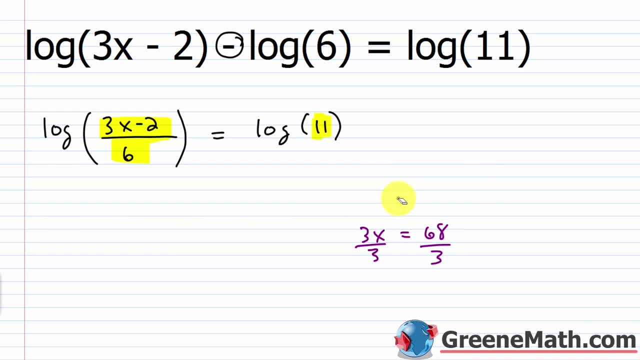 me kind of erase all this. So 68 is not divisible by 3. It's 17 times 2 times 2.. So we can just leave it as x equals. We'll say this is x equals 68 thirds. So in solution set notation we'll say 68 thirds And if you wanted to check that you could. 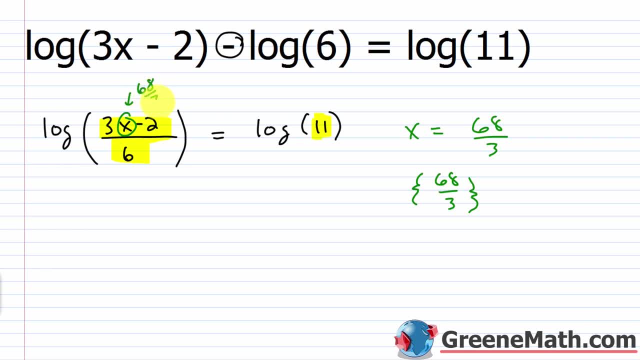 You could plug in a 68 thirds there and see what you get. If you plug in a 68 thirds, the 3s would cancel you. So you'd have 68 minus 2, which is 66.. 66 over 6 is 11.. So you'd have. 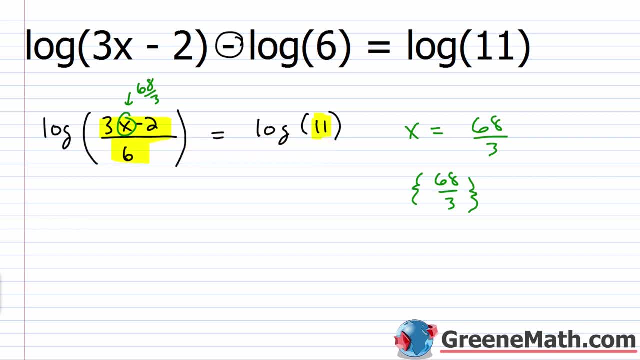 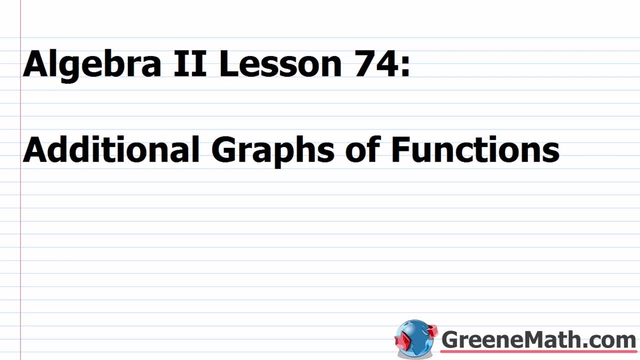 log of 11 equals log of 11.. That's true, So this does end up working itself out. Hello and welcome to Algebra 2, Lesson 74.. In this lesson we're going to look at some additional graphs of functions. So a few lessons ago we learned about graphing parabolas. Now, 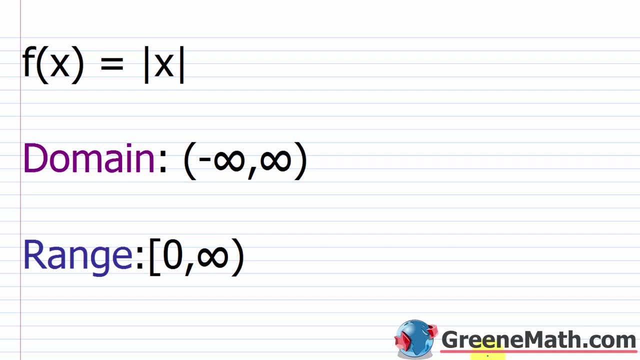 in that lesson we talked about the quadratic function f of x equals x squared, And then we compared other functions to that And we talked about the fact that we could have a vertical, a horizontal or both a vertical and a horizontal shift. So what we're going to do today is we're 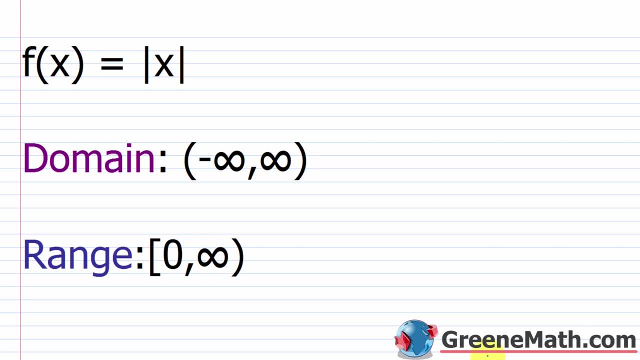 going to look at some other commonly occurring functions, things that you'll see in Algebra 1 and 2.. And we'll talk about what creates this vertical and horizontal shift And we'll talk about how you can determine if you have a vertical or horizontal shift without actually looking at. 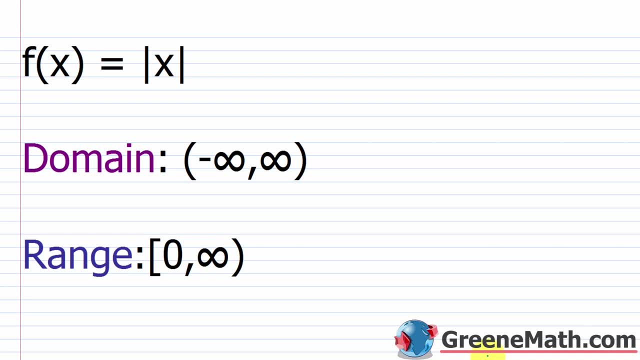 the graph or pulling out a t-table or anything like that. There's a very easy formula to follow. So the first one we're going to look at is the absolute value function We have. f of x equals the absolute value of x. When we talk about this function, the domain is any real number, So I can. 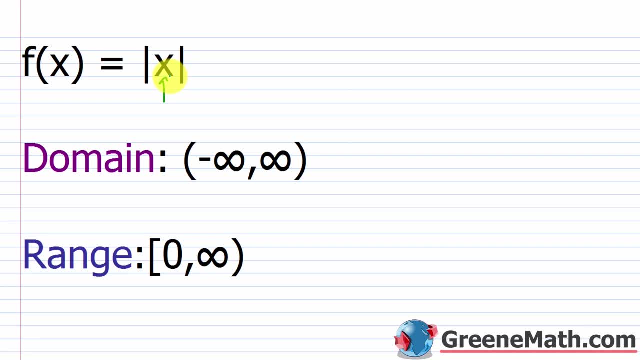 plug anything I'd like in for x, So I can plug anything I'd like in for x, So I can plug anything I'd like in for x. there I can do a negative, a positive, zero, whatever I'd like. The range is: 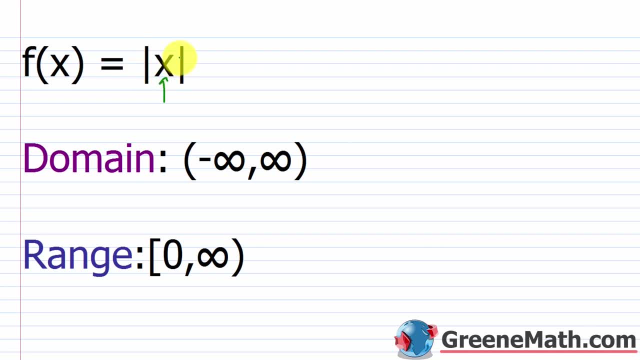 limited, though Remember the absolute value operation returns a positive if I plugged in a negative. So if I did something like the absolute value of negative five, that would give me an answer of positive five. If I did zero, I would get zero back. If I did a positive, I would get. 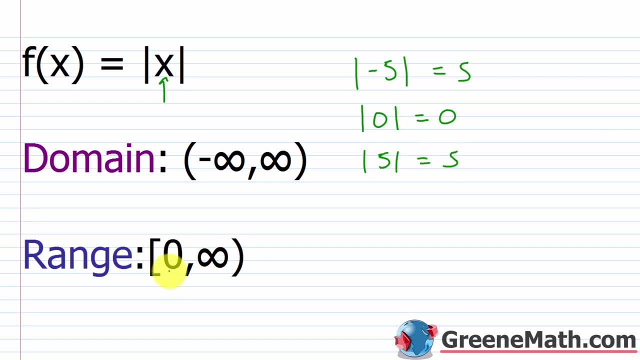 a positive back. So your range is limited. The smallest it can be is zero, The largest it can be is positive. So basically zero or any positive real number. Now one interesting thing: with the absolute value operation every number except for zero has an opposite, So five and negative five. 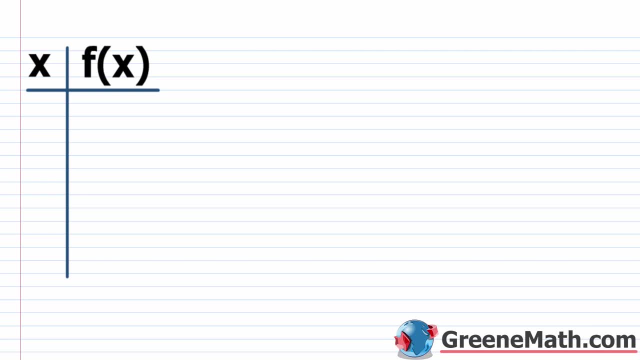 three and negative three. two million and negative two million Opposites have the exact same absolute value because, again, they're the same distance from zero on the number line. So what happens is you end up with a V shape when you graph this guy. In other words, if I was to 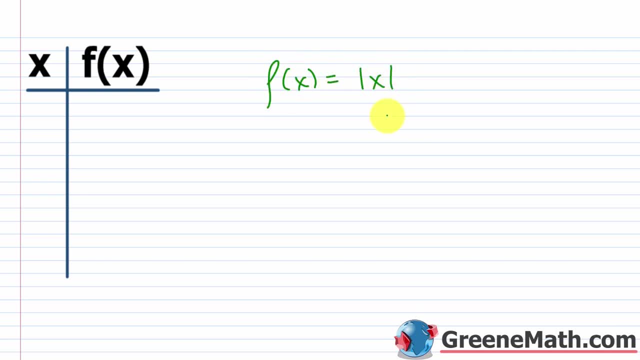 x-fy. if I were to have x as a plus or from limit, you would end up withation: times 보면, The entire answer is zero. So if I do a negative six and plus or minus negative zero, that is negative zero. How many people do I have to give my situations to Well after you? look at 1 minus 6, I know y equals 3.. Well, you have positive six. You can not always have negative six. So what we want to do is I'm going to look at the same values. I could do x equals e velio, or I'm going to do something over there that I get, So a negative 6. or a positive 6.. And what I want to do is I look at the same values of thecedo for x or six. they're independent, random five or they're semi- Tae. So my first thing is to go back to four, and then I'm going to try to solve the equation of the exercise. 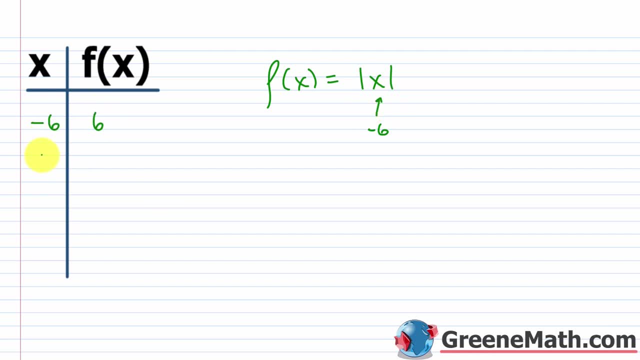 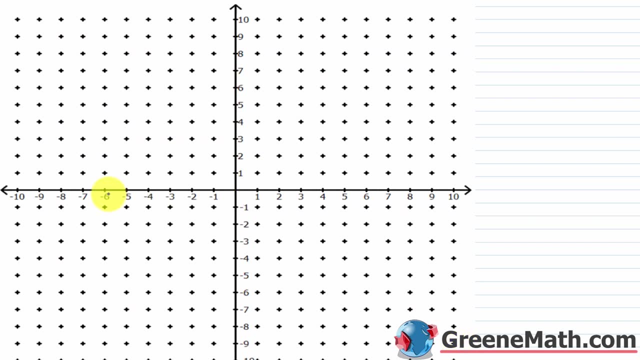 I would get positive 6.. Well then I could do an x value of 6 there and I would also get a y value of 6.. So if I look at my coordinate plane for an x value of negative 6, I'd have a y value of 6. 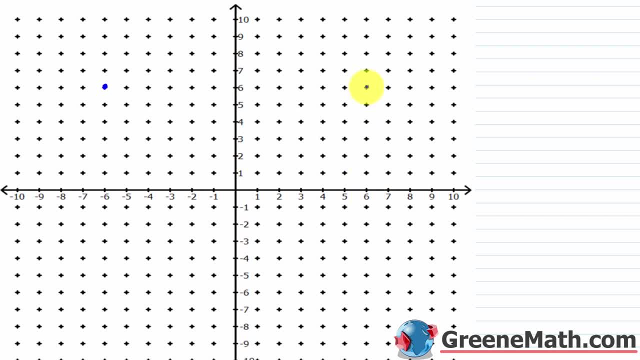 but also for an x value of positive 6, I'd have a y value of 6.. So this guy corresponds to here and here and what's going to happen is if I did an x value of 5, I would get a y value of 5. 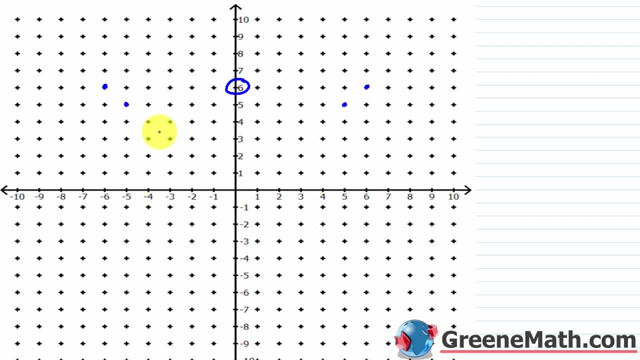 but an x value of negative 5 would give me a y value of 5.. So this keeps going down like this and it creates a v shape as it comes back up here. If you plugged in a 2 for x, absolute value of 2. 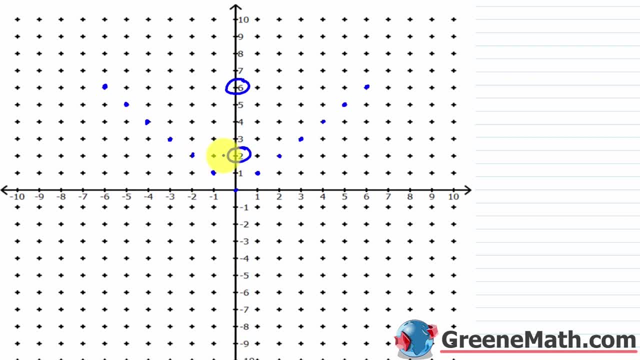 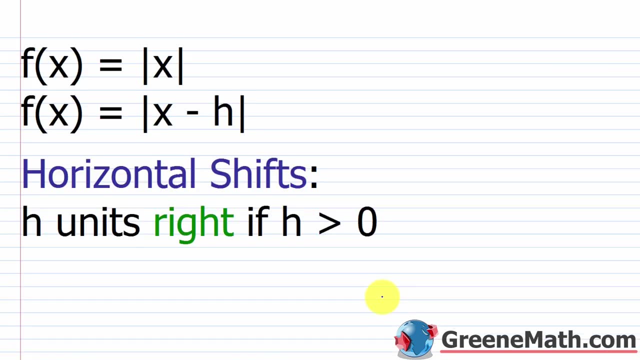 would give me 2. but if I plugged in a negative 2 for x, the absolute value of negative 2 would give me 2.. So let's graph this guy. Okay, so this is f of x is equal to the absolute value of x. All right, let's talk a little bit about horizontal shifts and I'll give 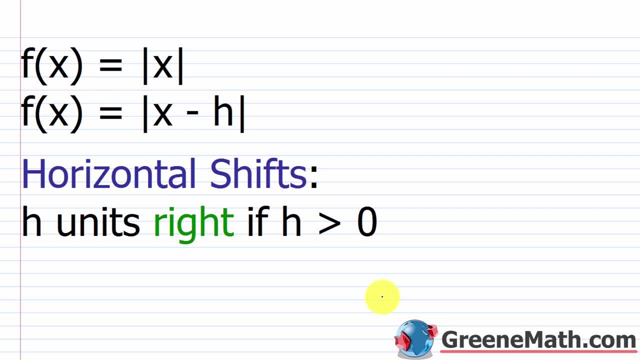 you a little shortcut here on how to tell if you have a horizontal shift and what the amount of the shift is, in which direction, and then in the example we'll get to in a second, I'll show you why it actually happens. So if you see, f of x equals the absolute value of x, and then you come. 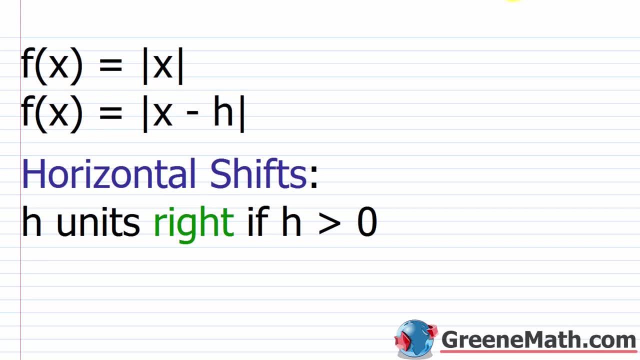 across f of x equals the absolute value of x minus h. the first thing you need to understand is that this minus h here happens inside of the absolute value bar, So we would say it happens inside of the function. So you want to write down in your notes that if 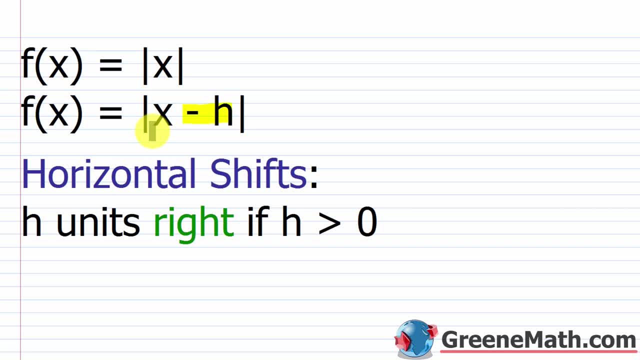 it happens inside of the function, you will have a horizontal shift. The way you can tell your operation, there is the absolute value operation. So if it happens inside of that, you're going to end up with a horizontal shift If it happens outside of it. so if you had f of x equals the 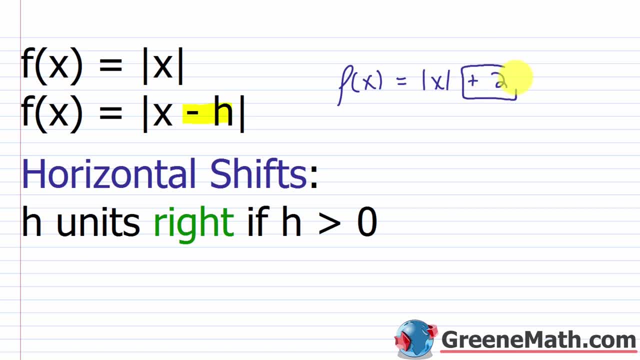 absolute value of x, let's say plus 2. this is outside of it. So this will be a vertical shift. but in this case it's going to be a horizontal shift. So if you have a horizontal shift and you have f of x equals the absolute value of x, you're going to have a horizontal shift. So in this case, 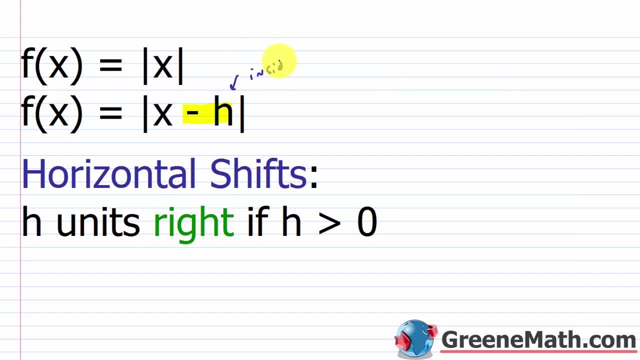 it's happening inside, So inside of the function. One way to tell for sure is to ask yourself: can I take this guy right here and plug it in for x in the original function, the one I'm comparing it to, would I get the same thing? The answer is yes, I would end up with this guy. exactly So it is. 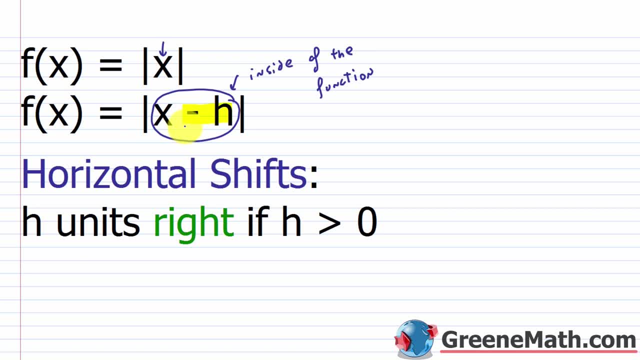 happening inside the function. we've established that Now, if you have something in this format, the horizontal shift will be the same as the horizontal shift. So if you have something in this format, the horizontal shift will be as follows: We say, if h is greater than zero, we would shift. 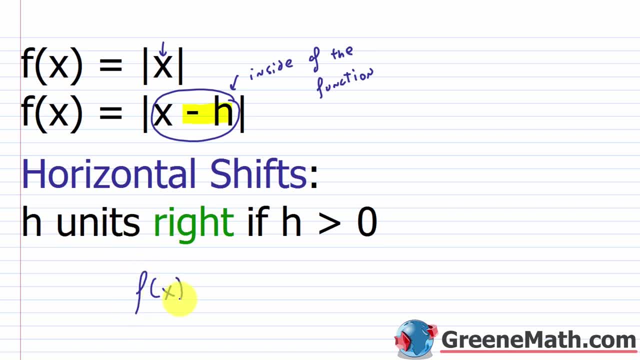 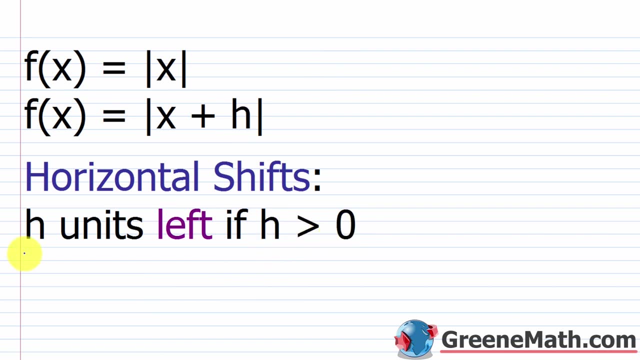 h units to the right. So if I saw f of x is equal to the absolute value of x minus 7, this would mean that I am shifting 7 units right, All right. the other scenario: if we have, f of x equals the absolute value of x plus h. here, if h is greater than zero, we're going to shift h units left. 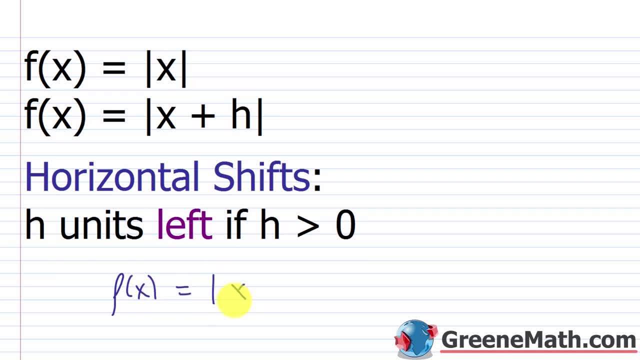 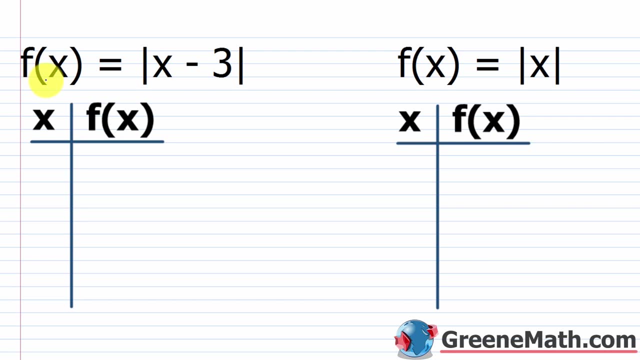 So f of x is equal to the absolute value of x plus 7. in this case, here 7 is greater than zero, so we would be shifting 7 units left. Let's think about why this is the case. Let's say again: compared to f of x equals the absolute value of x. we look at: f of x equals the absolute value of x. 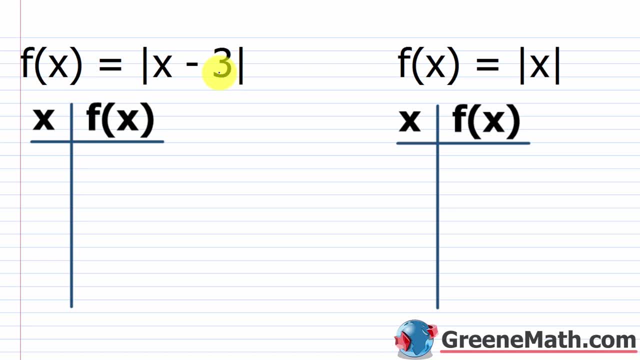 minus 3.. The shift, according to what I just told you, because this is a minus 3 here inside the absolute value operation- would be 3 units to the right. So this shifts 3 units right Now. why is that the case? Again, most of you will probably say it's a minus 3.. On the x-axis, if we're thinking, 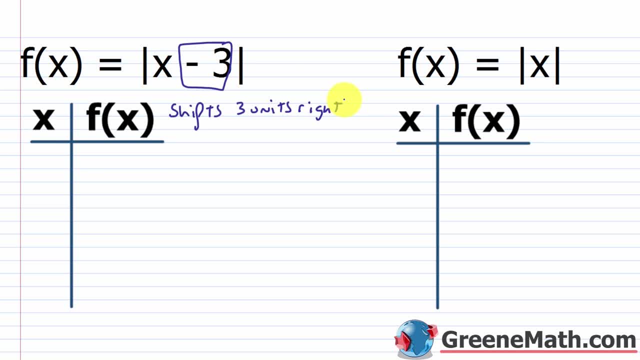 about that. a minus 3 would be 3 units to the left. So why is this guy saying 3 units to the right? What ends up happening is, for a given y value, a given vertical value on the coordinate plane, x now has to be 3 units larger to produce that. So let me show you with the t-table. 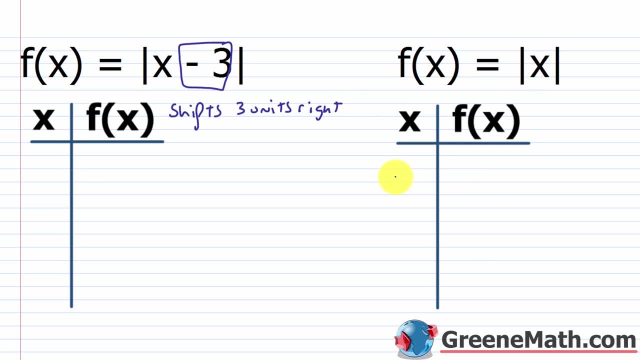 Let's say, in the original function I choose an x-axis, I choose an x-value of negative 3. I choose an x-value of 0 and I choose an x-value of positive 3. So the y-value here would be 3.. The y-value here would be 0 and the y-value here would be 3.. 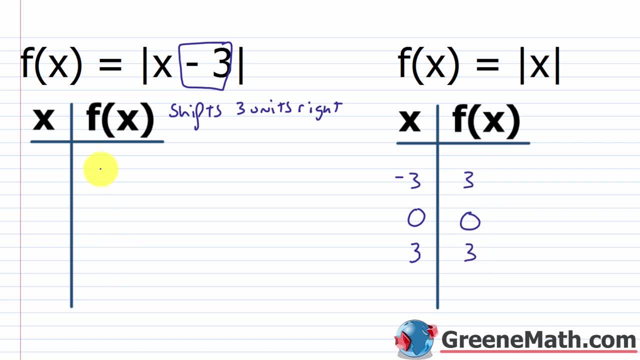 How can I get the same y-values over here? Let's just choose them already. So we're going to say 3, 0 and 3 is what we want. Well, I would have to plug in an x-value that's 3 units larger. 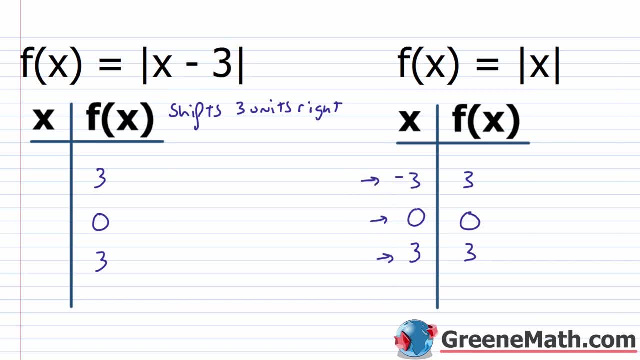 than these over here to compensate for this minus 3 here. So in other words, if I had a 0, which is 3 units larger than negative 3, the absolute value of negative 3 would give me 3.. So you see how, once I take away 3, I'm right back. 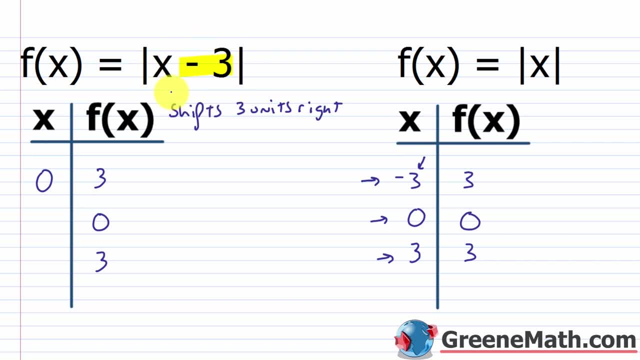 to this guy right here, and then I'm taking my absolute value. So I'm just kind of thinking about what amount would I have to put in there to kind of undo this operation of subtracting away 3, and that would give me the same result as I would have. 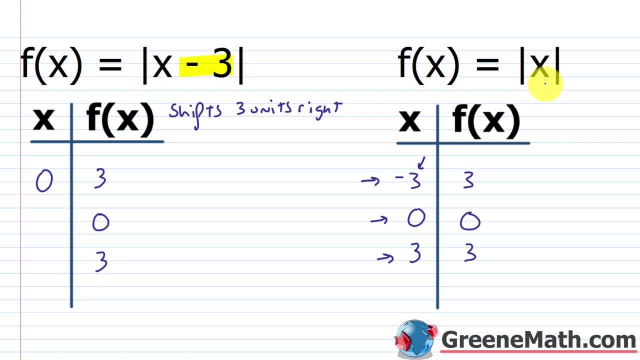 gotten if there was nothing done to it. Okay, so in this case I have to add 3 to undo the minus 3.. That's all I'm doing. So in this case, right here, if we have 0, we'd add 3. this would be 3.. 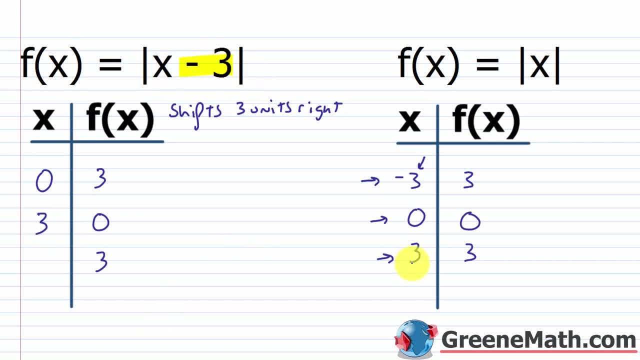 3 minus 3 would give me 0.. Absolute value of 0 is 0, and then, in this case, if it's 3, it would go to 6.. 6 minus 3 is 3.. Absolute value of 3 is 3.. So that's all we're really doing: We're adding 3 to. 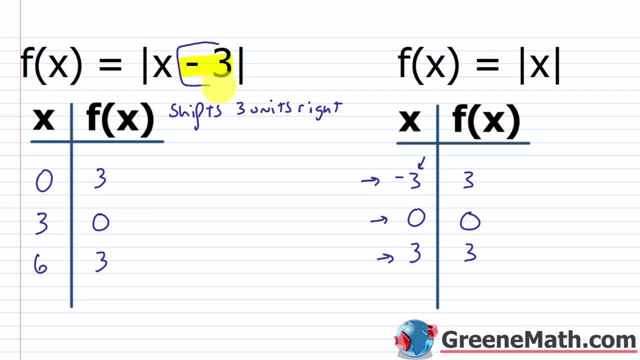 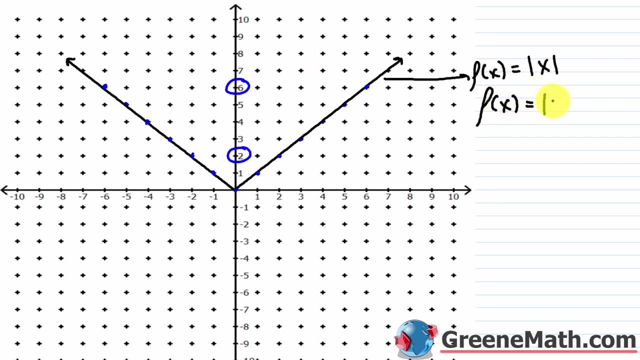 each x-value to undo the effect of this minus 3.. So if we looked at a graphso we did, f of x equals the absolute value of x minus 3.. Some points we looked at so far were 0 comma 3, 3 comma 0, and 6 comma 3.. So 0 comma 3. 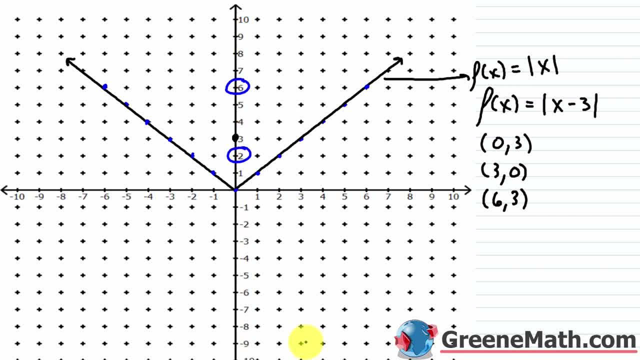 is going to be right here, Then 3 comma 0 is going to be right here and 6 comma 3 is going to be right here. So all we're really doing is shifting everything to the right three units. so this would go three units to the right. 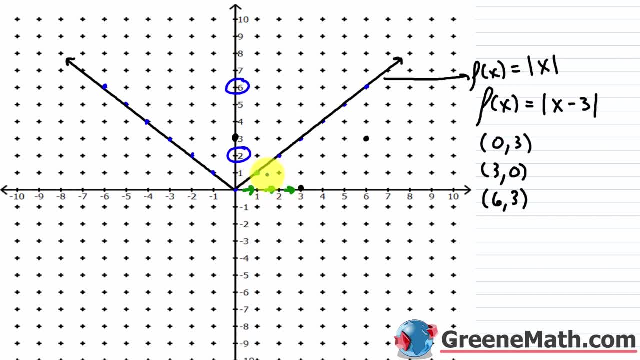 that's my point. I could take this point right here and go one, two, three years to the right. that would be my point. I could take this guy one, two, three years to the right. that's my point. one, two, three years to the right. I already have it: one, two, three years to the right. you know so. 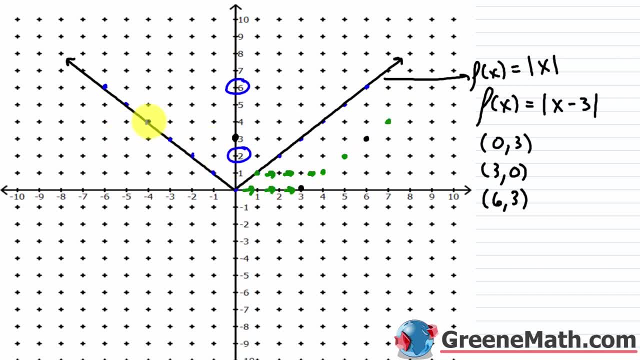 on and so forth. it's the same thing with these points over here. so I could take this one and go one, two, three units to the right, this one, one, two, three units to the right, you know, so on and so forth. so this guy, let me label it this is: f of x equals the absolute value of x minus three again. 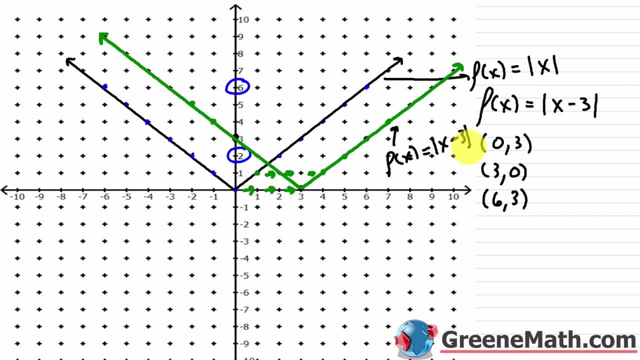 for a given y value, the x value now has to be three units larger, and so that creates a graph that's just going to shift to the right by three units. so hopefully that makes some sense for you again. a lot of people think that minus three would cause you to go to the left by three, but 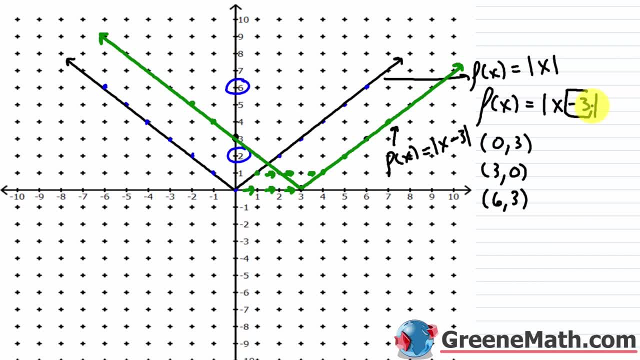 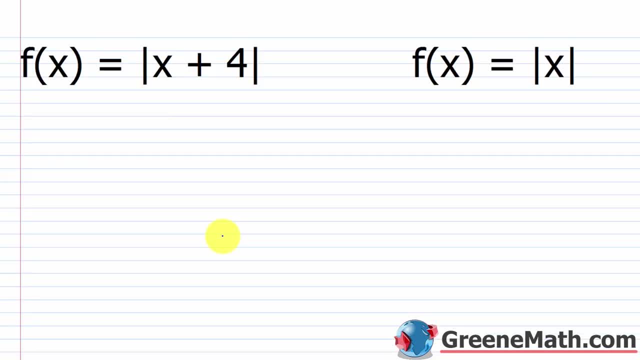 it's the opposite of that. you want to go to the right because you're trying to undo the minus three, so you basically have to think about it as i'm adding three, so i'm going to the right by three units, all right. so what if i saw? f of x equals the absolute value of x and compared to that i have f. 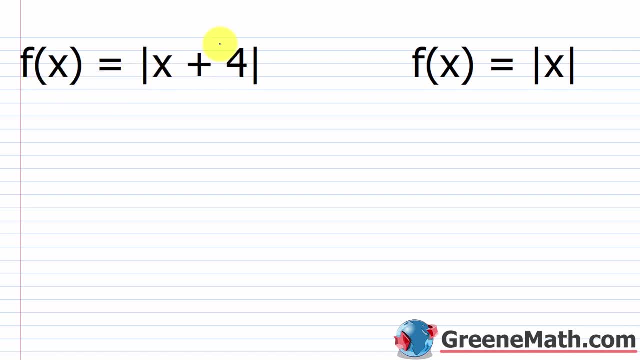 of x equals the absolute value of x plus four. well, in this case i'm adding four. so again, if i just think about it simply, what do i need to do to undo the addition of four? i would subtract four. so that means i'm shifting four units to the left. so i shift. or i could say: 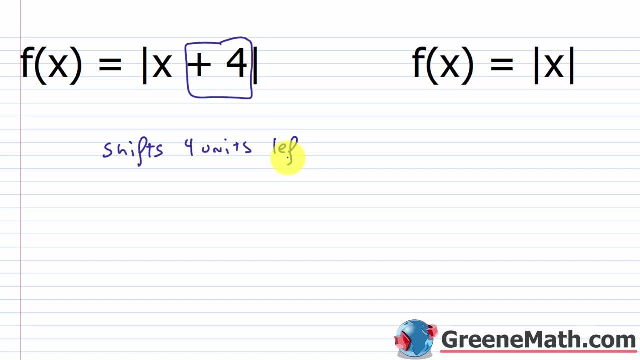 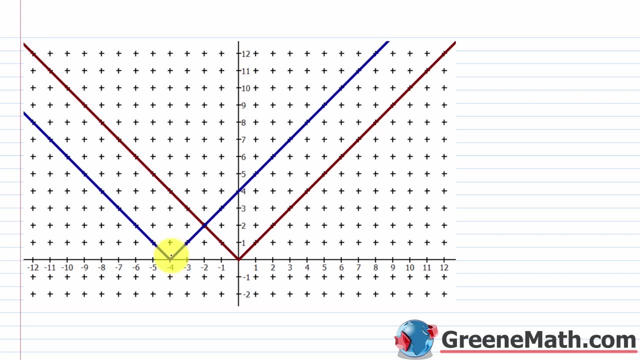 shifts four units left right, pretty easy. so i have this guy drawn already for us. here's the original and then here's the other guy where we have f of x plus four. you can see every point has just moved four units to the left, and again that's to compensate for the fact that we're adding four to x. 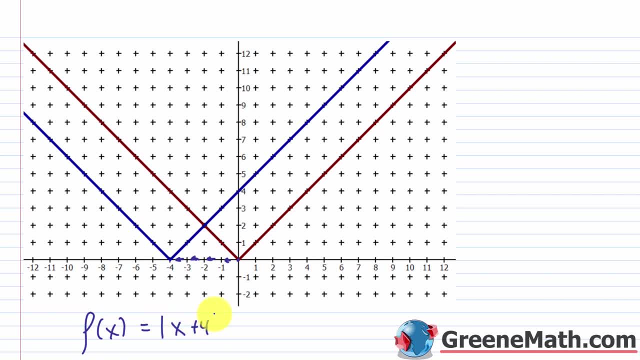 for example, if i have f of x equals the absolute value of x plus four, to get a y value of zero i now have to plug in an x value of negative four to undo that plus four. there negative four plus four would be zero absolute value of. give me zero. so to get a y value of zero now my x value has to. 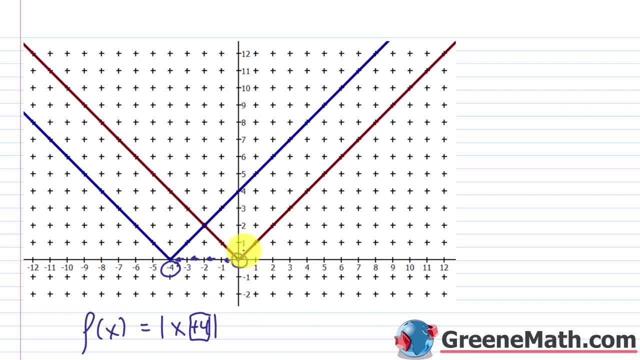 be negative four, whereas before my x value was zero. so everything just shifts four units to the left to compensate for that plus four. that's inside the absolute value operation, so i'm going to plug in a negative four. that's inside the absolute value operation, so i'm going to plug in a negative. 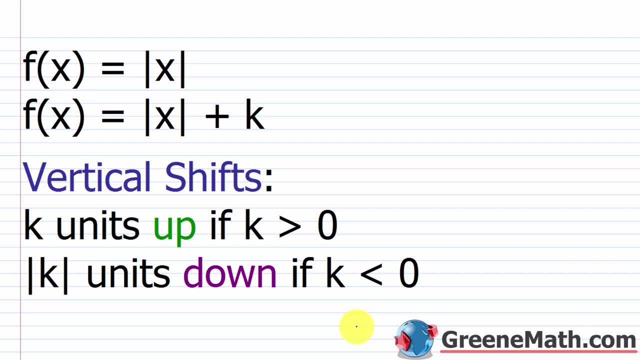 four, that's inside the absolute value operation. all right, so the next thing we want to talk about would be a vertical shift. so if we're looking again at, f of x equals the absolute value of x, and we see f of x equals the absolute value of x plus k. well, now what's going to happen is for a 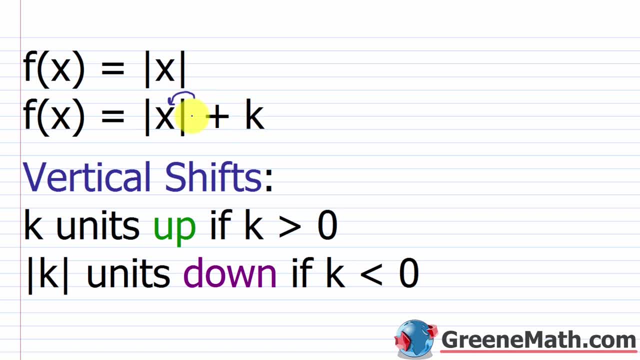 given x value, i plug something in for x, i take the absolute value, everything is the same. but then i have this plus k that gets tacked on to the operation. so my f of x or my y value will change based on this. so this is going to directly affect y, and when we affect y we're affecting the vertical axis. 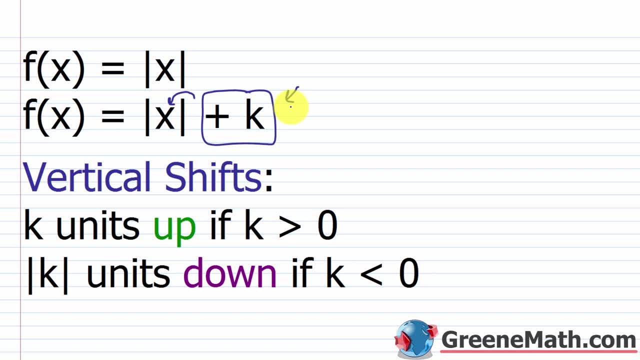 so we're going to shift up or we're going to shift down. so if k is greater than zero- meaning i had something like f of x equals the absolute value of x plus, let's say, three- well, in this case k is greater than zero. we would just say that we're shifting up by three units. in the case where k 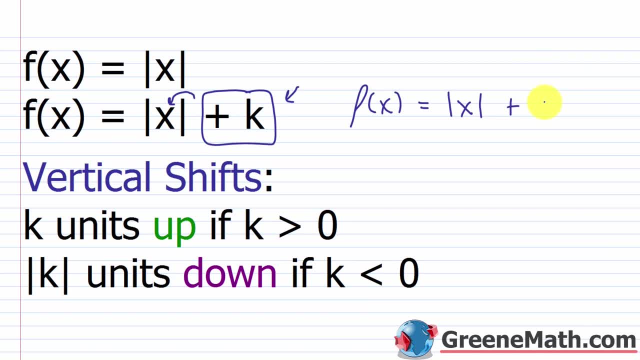 is negative. so let's say this was plus negative three. well, in this case we're going to shift up by three units. so we're going to shift up by three units. in this case we're going to shift the absolute value of k units down, so the absolute value of 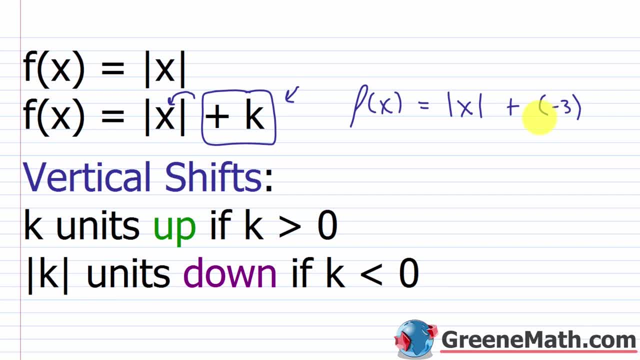 negative 3 is 3. we'd say we shift three units down. now no one would ever write it like this. this is just how it is presented in your textbook in most cases. you just see minus 3 here. so you would just kind of adapt and say, okay, i know, if i'm subtracting away 3, i go down 3. if i add 3. 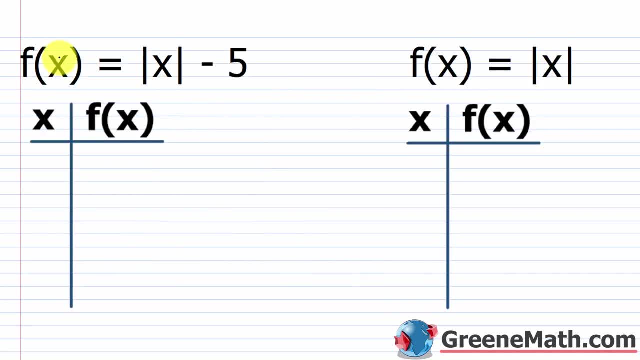 i know i'm going up by three. all right, let's take a look at an example. so we have f of x equals the absolute value of x minus 5, and we have f of x equals the absolute value of x. so We can say: for a given X value, the Y value that will be produced will be five units less. 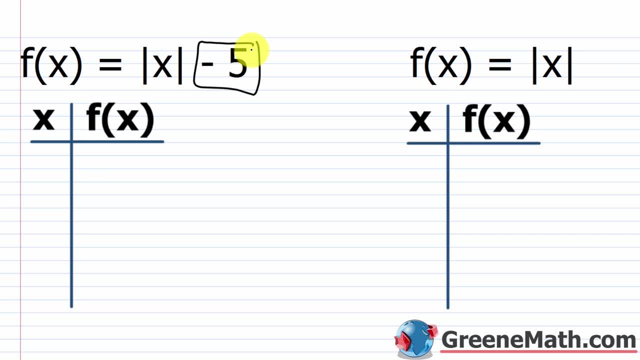 And this will create a vertical shift down by five units. So again we can go with negative three, zero and three. This would give me three, zero and three For this guy. if we have negative three, zero and three, again I plug in a negative three here. 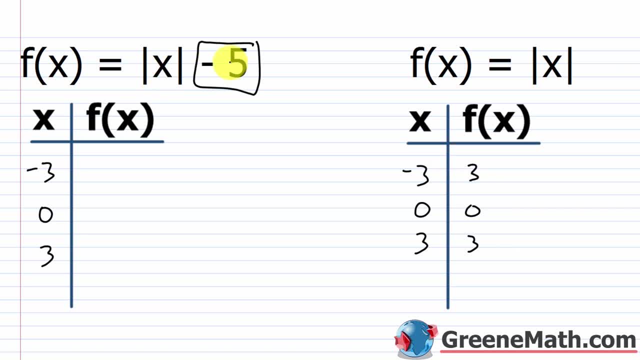 I take the absolute value, I get this result, but then I just get minus five. So I can basically take these values and subtract away five and give myself the Y value from over here. So three minus five would be negative two. Zero minus five would be negative five. 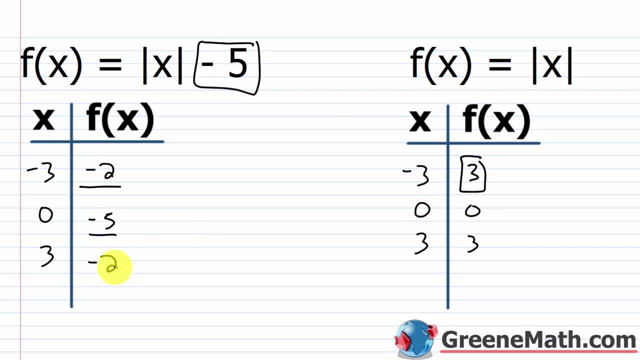 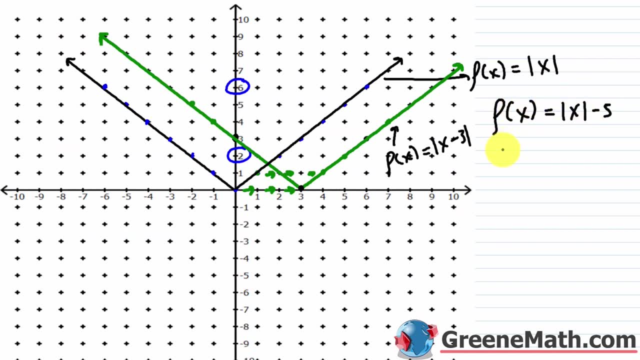 Three minus five would be again negative two. So I can take these points and plot them. So we have: F of X equals the absolute value of X minus five. Our first point: we have negative three comma negative two. We have zero comma negative five. 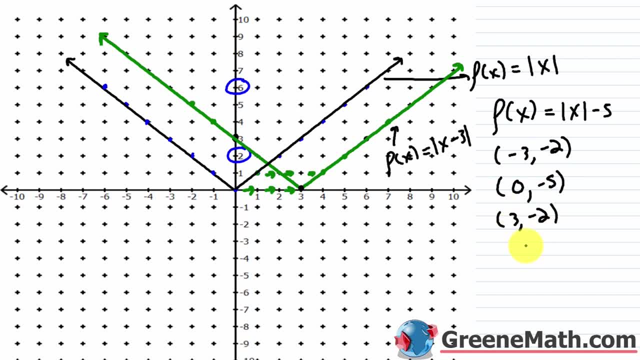 And then we had three comma negative two, So negative three negative two. It's right there. We have zero comma negative five And we have three comma negative two, So three negative two. Now I can just take points from this original guy and shift them down five units if I want more. 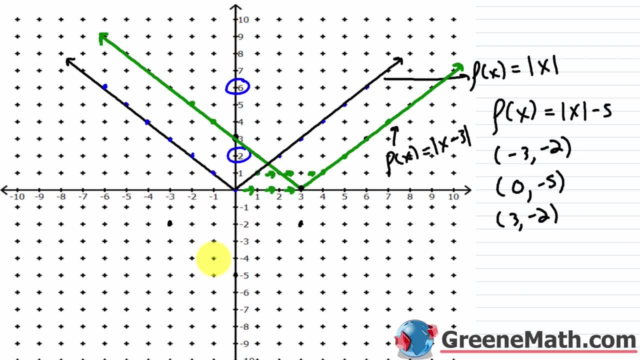 So I can take this point and go down one, two, three, four, five. I can take this point and go down one, two, three, four, five And you can see where the line is. This right here would be the lowest point on the graph. 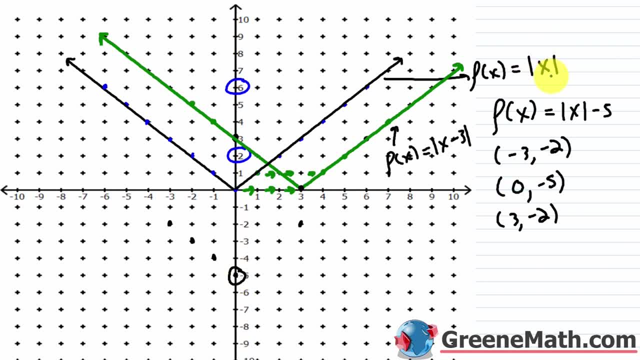 We know that right, Because if X is zero, that's the lowest I can make this guy, Because the absolute value operation: if you plug in a zero you get zero. If I plug in something negative, remember I'd get a positive. 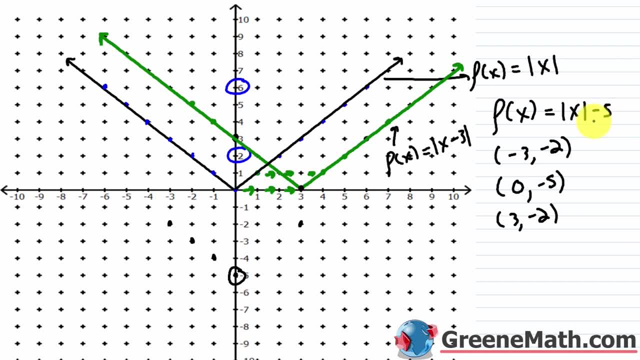 So the lowest I can get is if X is zero, That gives me a Y value of negative five Over here. if I shift some of these down, if I take this guy and go down one, two, three, four, five, 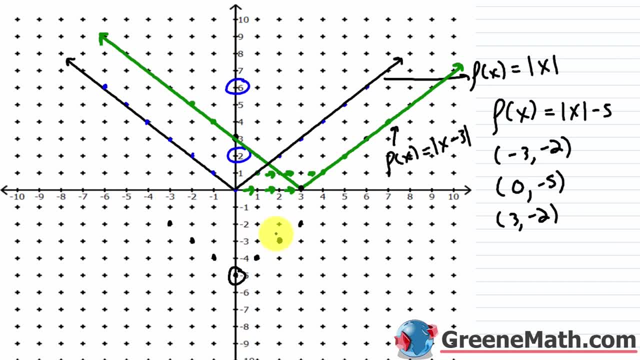 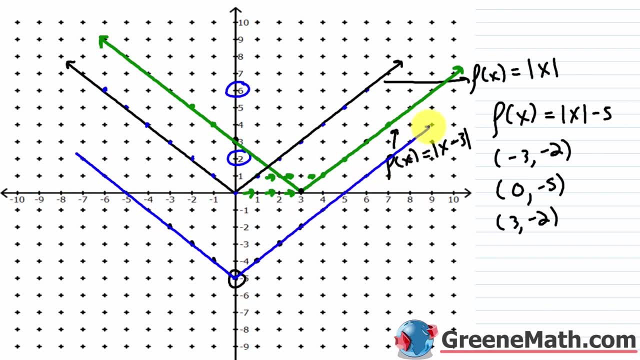 Over here: one, two, three, four, five, And I have enough points to get a good graph going. Okay, so this would be my graph, for F of X equals the absolute value of X minus five. So again, every point on the original is just shifted down five units. 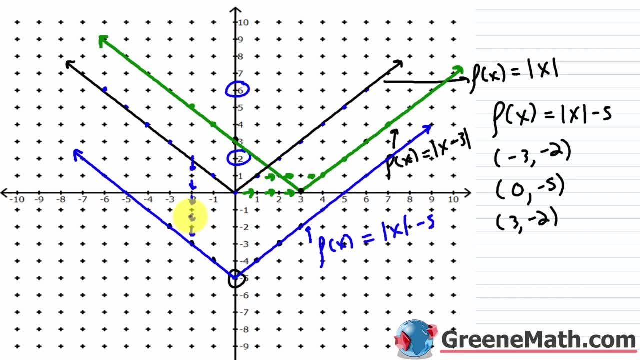 So this went down: one, two, three, four five. This one went down: one, two, three, four five. This one went down one, two, three, four five. You know, so on and so forth. 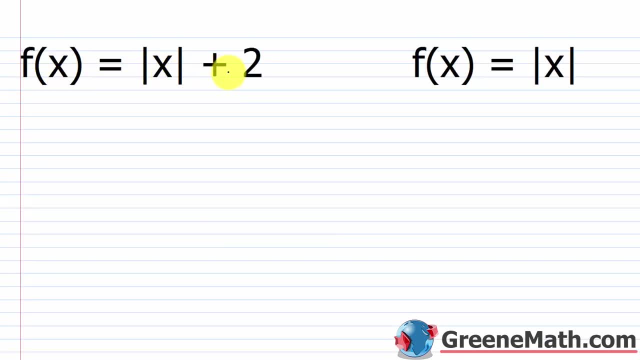 So in this next example we see: F of X equals the absolute value of X plus two. So now I'm adding two outside of the absolute value operation. So again I'm just shifting the graph up by two units. So we can say this shifts two units up. 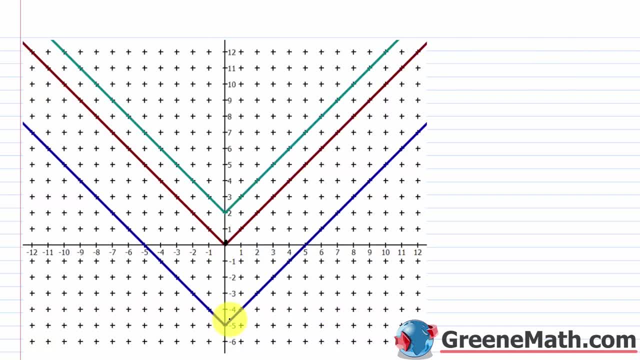 So here's all three of these guys. Here's the original, Here's the guy that was shifted five units down And here's the guy that shifted two units up. Right, so if I plugged in a zero for X, obviously I'm going to get zero for X. 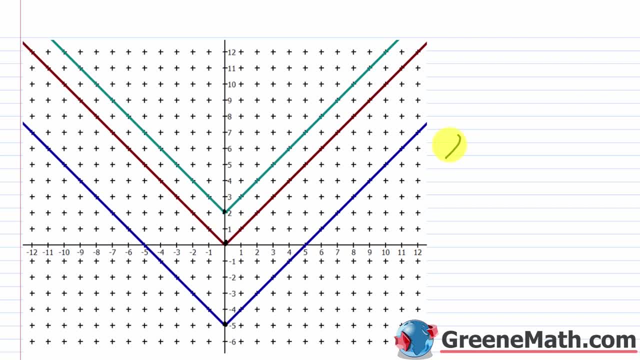 So basically you would get two for Y, right, Because you have F of X equals the absolute value of X plus two, So you get a zero there. Zero plus two would give you two. So everything is just shifted up two units, as we would expect. 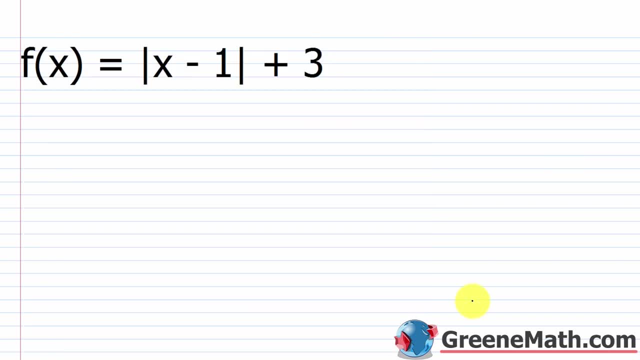 So what happens if they throw both of these on you? So, in other words, you get a horizontal and a vertical shift. This part right here happens inside the absolute value operation. This part right here happens outside. So this will create a horizontal shift. 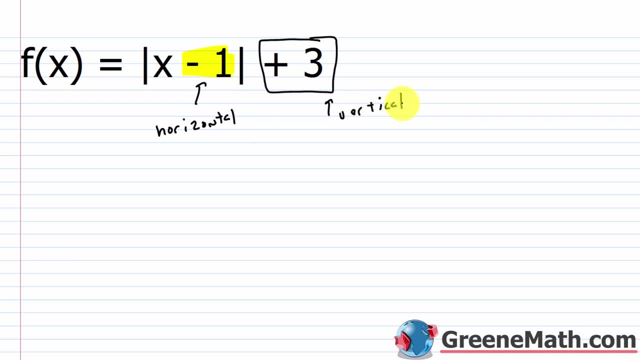 And this will create a vertical shift. You just have to remember: inside the function or inside the operation is giving you a horizontal shift, Outside is giving you a vertical. So with a vertical shift, it's intuitive. So if you're adding something, you're going up. 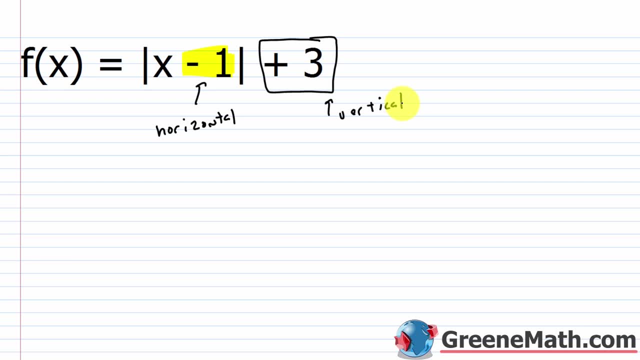 With a horizontal shift. it's counterintuitive. If I'm subtracting, I'm going to the right. So if I have X minus one, Here again I've got to think about what can I do to counteract that minus one. 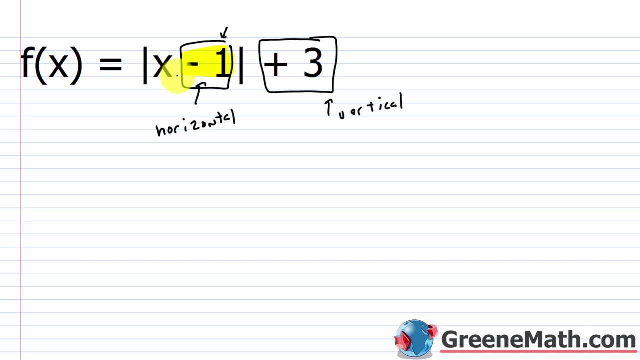 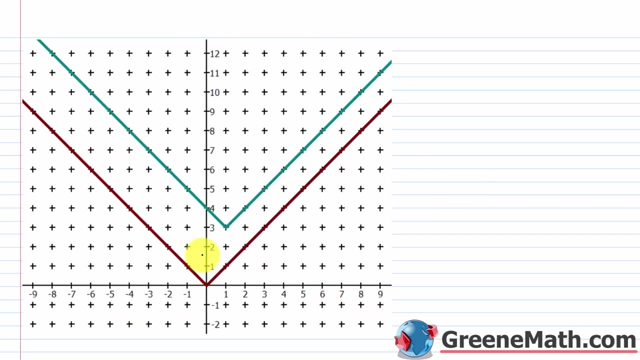 How can I get this back to where it was? I've got to add one. So I'm shifting to the right, So this shifts right by one unit And it's going to go up by three, Up by three units. So here's a graph of, again, the original. 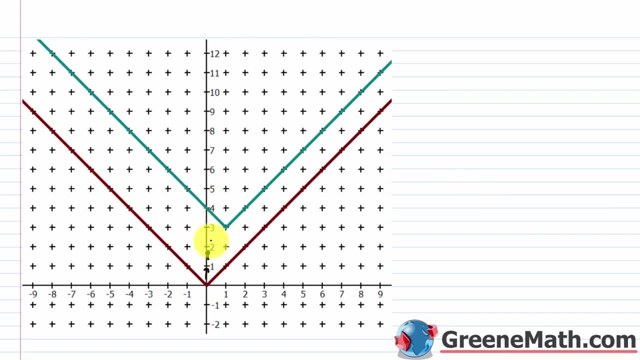 Here's a graph of the guy that shifted. So it went up one, two, three And to the right one. So there's your new lowest point And you can take any given point and go up three units and to the right one. 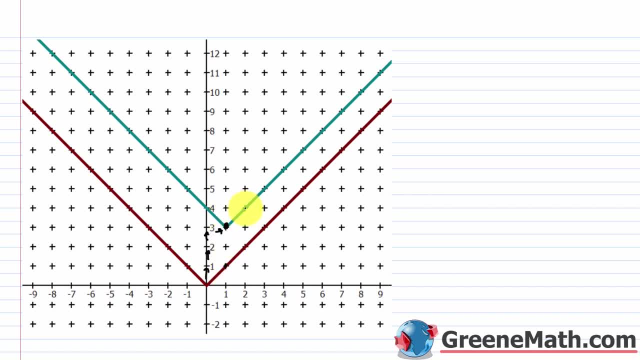 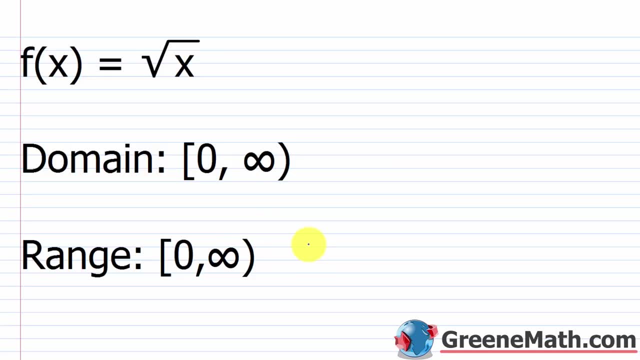 You'll be on the new graph, So you'll go up one, two, three to the right one. You can take this point and go up one, two, three to the right one, So on and so forth. All right, the next function we're going to talk about is the square root function. 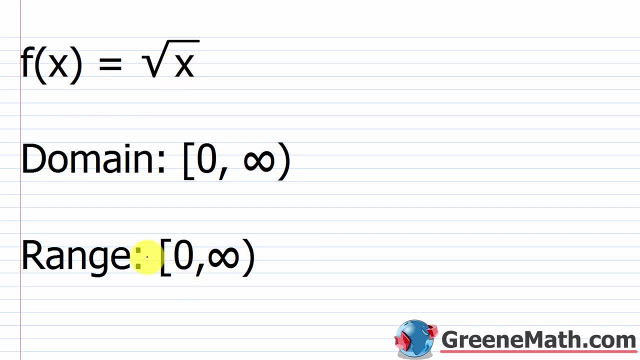 So we have: F of X equals the square root of X. The domain and the range for this guy are both limited, And the reason for that is simple: If I plug something in for X here, I can plug in a zero. square root of zero is zero. 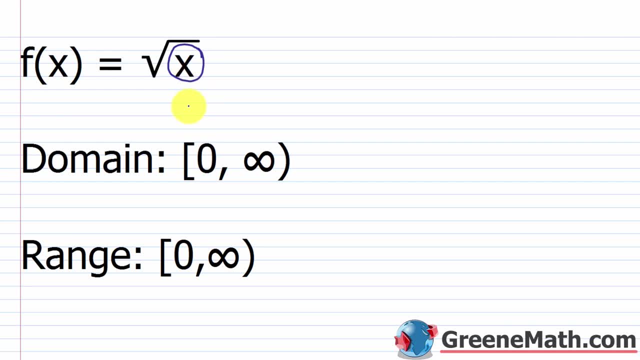 I can plug in a positive square root of positive will give me a positive. But remember, I can't take the square root of a negative number without involving the imaginary unit or the complex number system, Because we're eliminating this to the real number system. we would say our domain is. 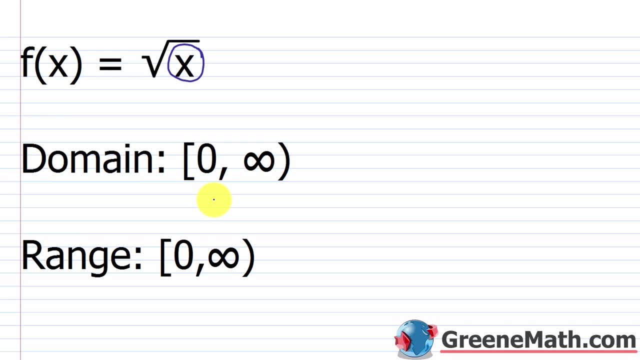 restricted to zero or anything larger, And the same thing for the range zero or anything larger. All right, So if the function we're comparing everything to is again, F of X equals the square root of X, For F of X equals the square root of X minus three. 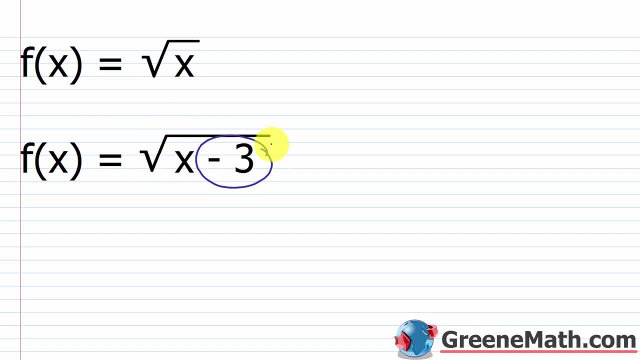 This is happening inside the function, inside the square root operation. So if it happens inside the function, we have a horizontal shift And again it's going to be counterintuitive. So what do I need to do to cancel out this minus three here? 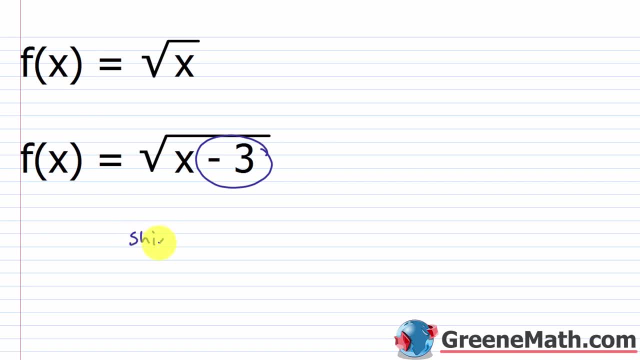 I would add three. So you think about it like that: This is going to shift where you could say: shifts three units, right? Because again, Okay, So we're given Y value, My X value now has to be three units larger to compensate for this minus three here. 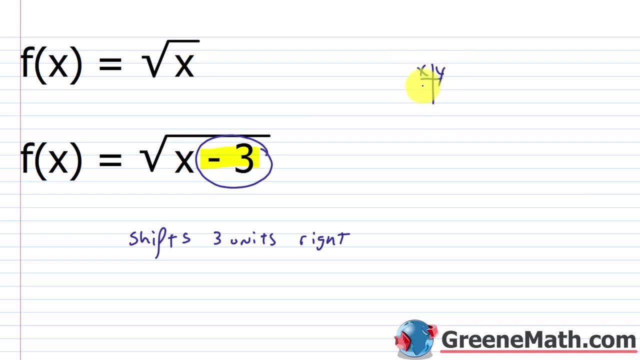 As an example, let's say we looked at one ordered pair. Let's say I plug in a zero for X. I know I would get a zero for Y. Well, here, to get that Y value of zero, what would X have to be? 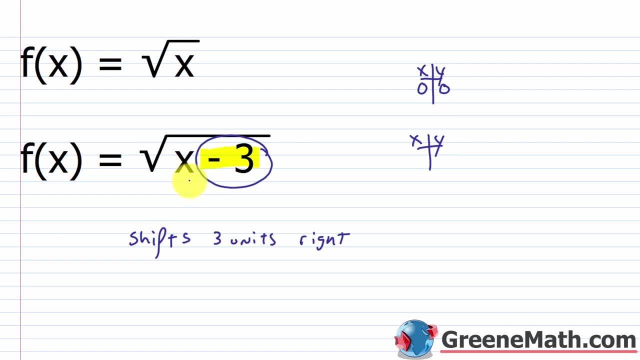 I would have to increase it by three units. I would now have to plug in a three for X. Three minus three would give me zero. Square root of zero would give me zero. So a three for X would now give me a Y value of zero. 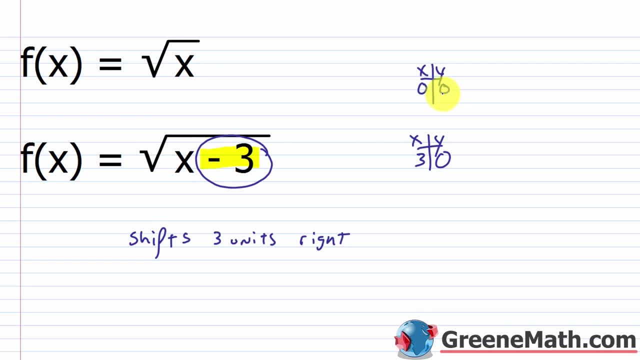 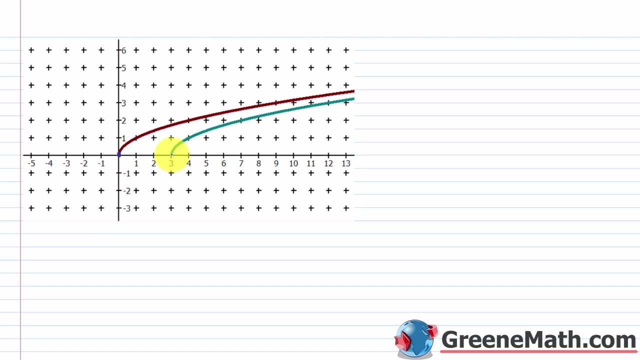 Whereas before an X value of zero would give me that same Y value of zero. So I had to increase X by three units and it would be the same thing everywhere. I'm just shifting the original graph three units to the right. So if we look at the graph, here's the original. 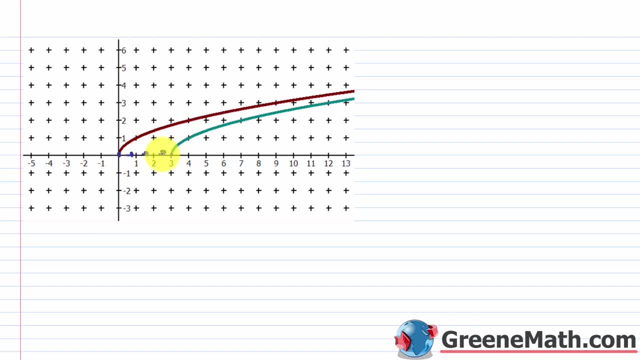 Here's the one that we looked at after. So everything is just moving three units to the right. Here's another point. here This goes: three units to the right, Okay, Three units to the right, you know. so on and so forth. 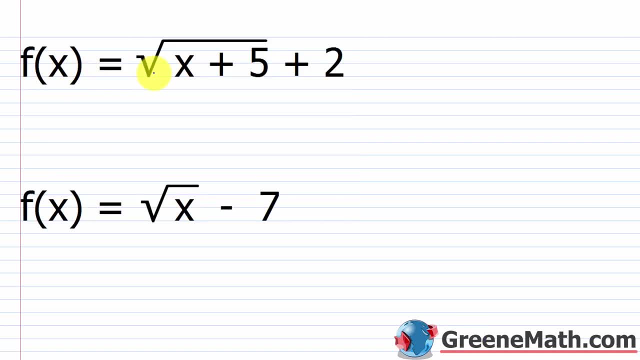 All right, Let's take a look at some more here. So we have: F of X equals the square root of X, plus five, then plus two. So you have two different things going on. You have something inside the function and something outside the function. 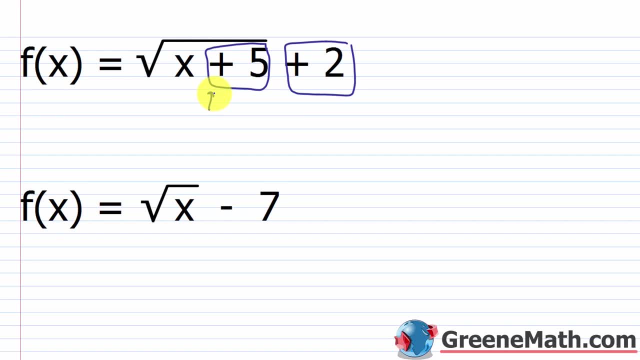 So inside the function you have plus five. So again, to undo that adding of five, I've got to subtract five away. So that means I'm going to shift to the left by five units. So this shifts left And then I have plus two. that's happening outside the function. that would just drive. 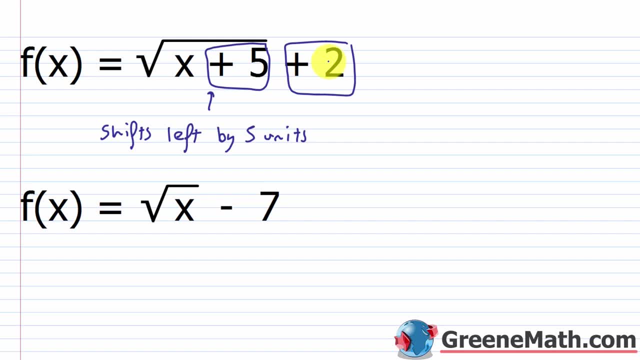 up my Y value by two for a given X value. So this would cause it to shift up by two units. So, and up by two units, then we have F of X equals the square root of X minus seven. This is happening outside the function, outside the square root operation. 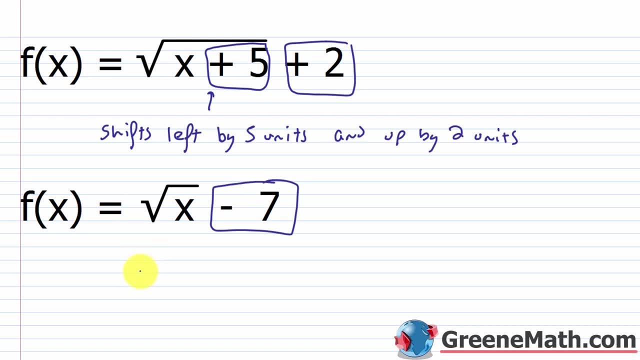 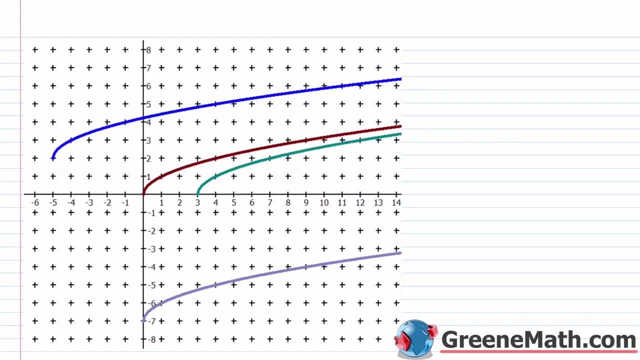 So we can just say: this shifts down by seven units. So this shifts down by seven units. So here's all your graphs drawn, if you wanted to look at them. Here's your original, Here's the one that was shifted down by seven units. 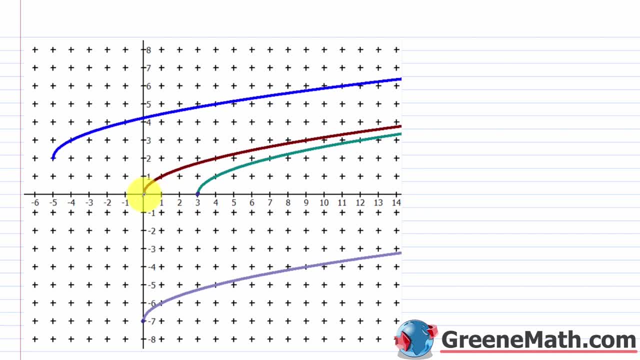 Here's the one that was shifted to the right: three units. And this guy had both changes right. It was shifting horizontally and vertically, So it went up one, two units and it went to the left one, two, three, four, five units. 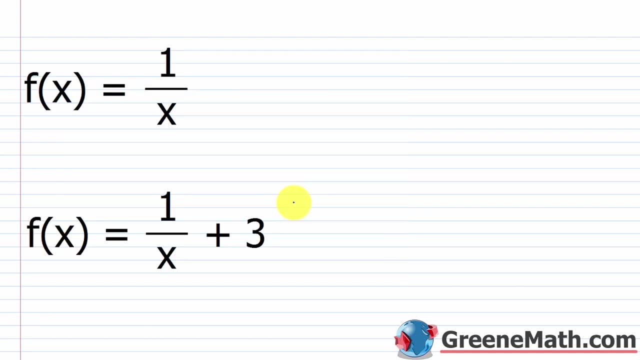 All right. So the next function we're going to look at is known as the reciprocal function. So we have F of X equals one over X. The domain and range I haven't listed here, but essentially the domain is anything but zero. I can't plug in a zero because I don't want to divide by zero, and my range is also anything. 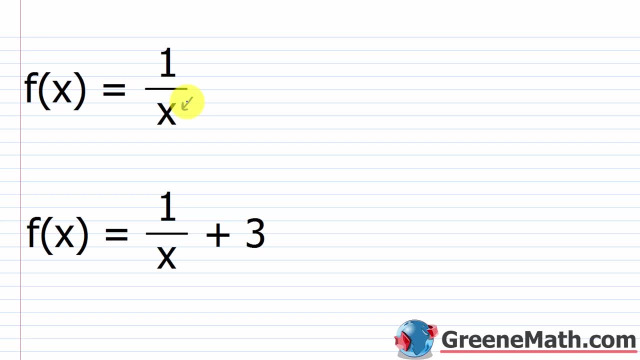 but zero. So any number in the real number system you choose, other than zero, is allowed. So the first thing, we'll compare to it. we have: F of X equals one over X plus three. This is happening outside. This is happening outside of the function. 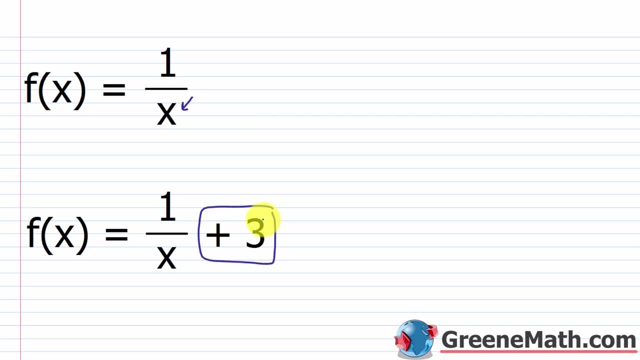 So if it happens outside of the function, it's a vertical shift. In this case we're just going to move up by three units. So we'll say this shifts up by three units For a given X value. you could see the Y value would just increase by three. 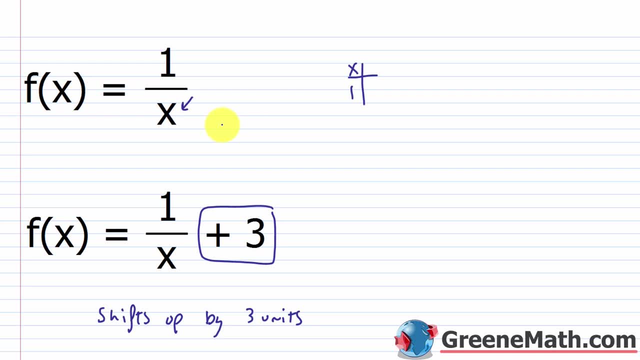 If, in this one, I chose an X value of one, to make it really easy, my Y value would be one. right Plug in a one there. One over one is one, So Y is one. In this case, if I chose an X value of one, my Y value, according to this, should be four. 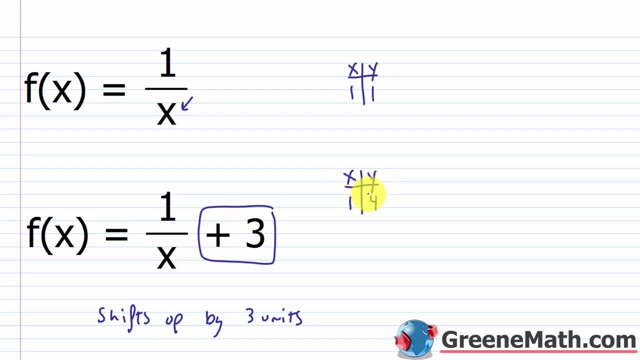 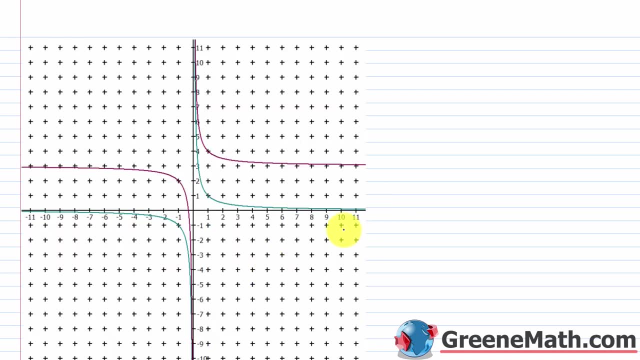 One over one would be one. One plus three gives me four. So that's what I would have. So every point just shifts up by three units. So here's a graph of these guys. You can see if you pick a point like one comma one on the original, you can just shift it. 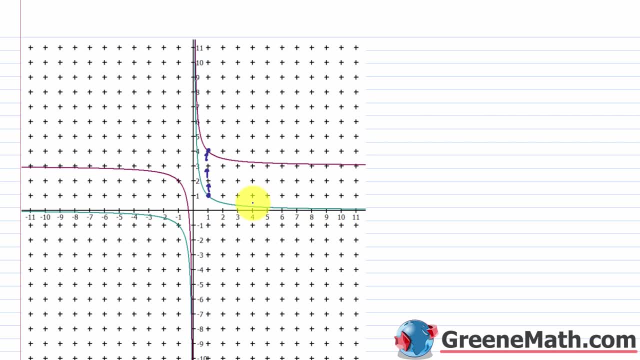 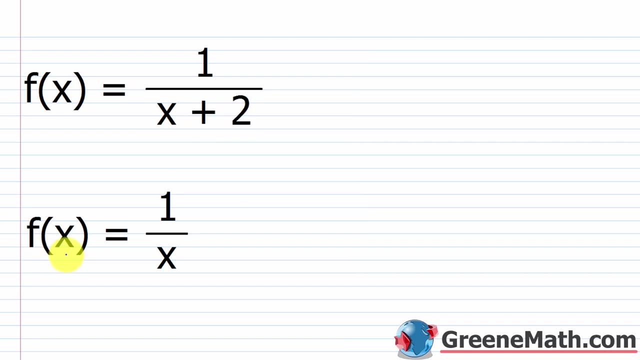 up by three units and you get to it on the other one. So everything has just moved up again by three units. What about? F of X equals one over X. F of X equals one over X plus two, Again, compared to F of X equals one over X. 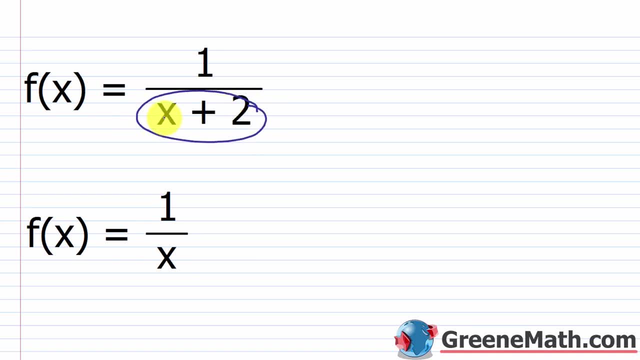 So this part right here is happening inside the function. I could take X plus two and plug it in for X. So what happens is that's going to give me a horizontal shift. So if it's plus two here, you just think about the fact that I would need to subtract two. 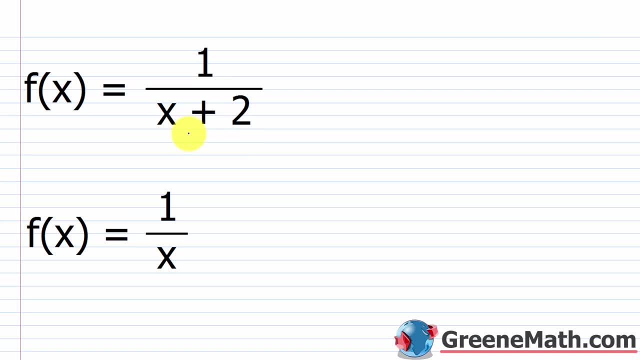 away to bring it back to where it was. I'm thinking about how I can counteract that plus two there. So, for a given Y value, my X value needs to be one. So I'm going to do that. Okay, So I'm going to do this. 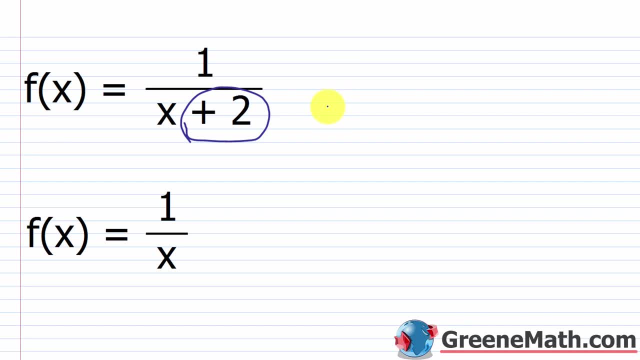 And I'm going to do the following again, I'm going to do like this. So I need to be two units smaller to get to it. So I would say: this shifts two units left. And to prove that to you again, let's do a little T-table. 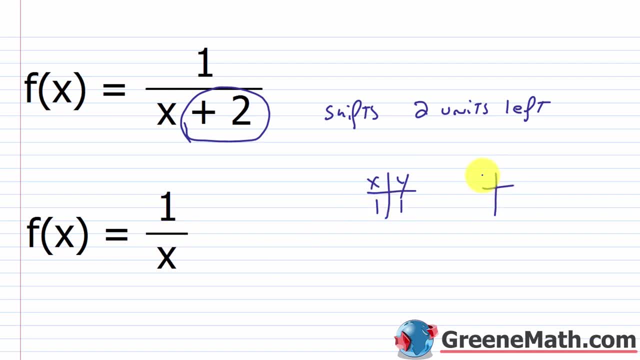 I know in this guy I could do one comma, one as a point Over here. according to what I just said, the X value would now need to be two units less. So that would give me an X value of negative, one that would produce a Y value of positive. 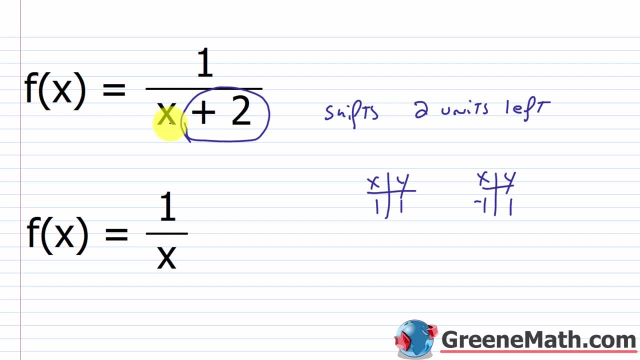 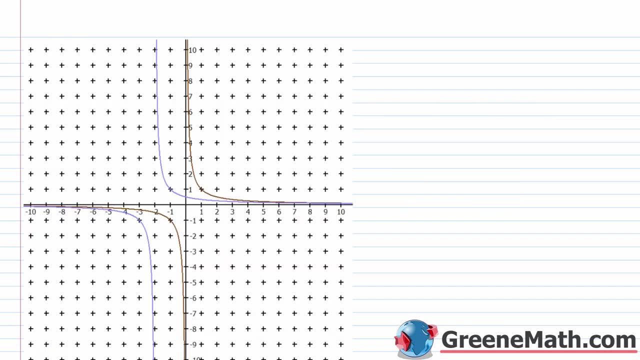 one, And let's try it. If I plug that in a negative one, it would produce a positive one. a negative one there. Negative one plus two would give me one. One over one is one, All right. So here's the two graphs drawn for you. This is the original. You can see that point right there. 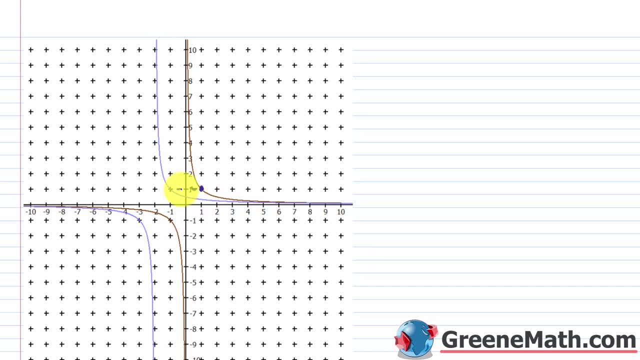 one comma one, And again it's just shifted two units to the left. So there's your new point where you have negative one comma one. So every point in that original would just shift two units over to give you the new function graph. All right, So the last function I want to cover today. 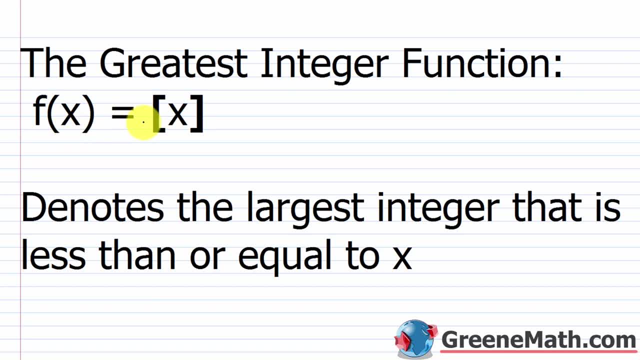 is called the greatest integer function. So this guy, f of x equals the greatest integer of x. You might also hear this called the floor function. Now, the notation for this guy varies greatly. You might see brackets around x like this. You might see kind of L-shaped brackets. 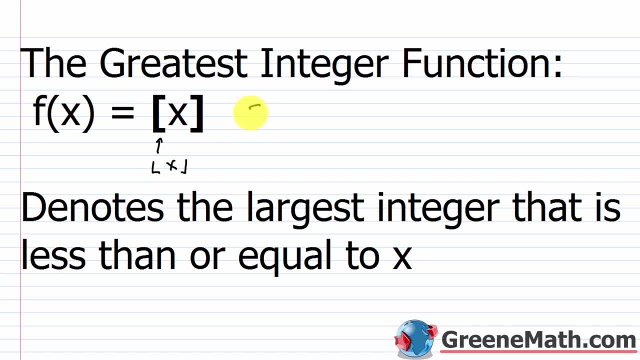 like that. You might also see something that looks like this. This is very common. You probably see that in your textbook. It's in the textbook that I'm using to write this lesson, So no matter what you see, it all means the same thing. In your calculator, you'll probably see int and then x. 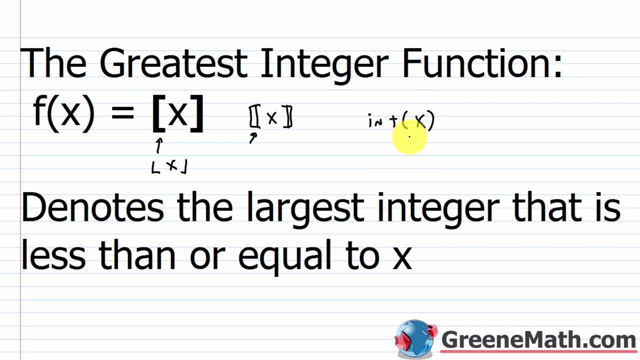 like that All means the same thing. What this denotes is the largest integer that is less than or equal to x. You got to think about this as it rounds down to the nearest integer. So if you're at an integer value, you stay there. If you're not at an integer value, you're rounding down. 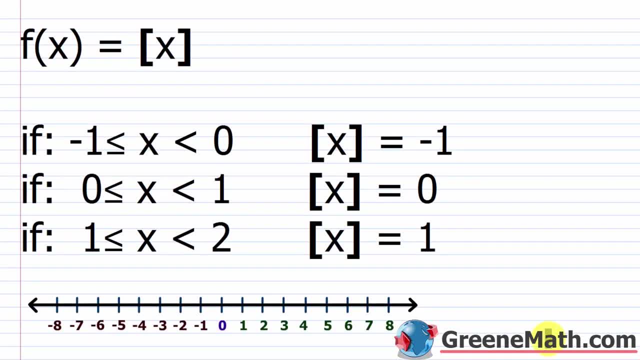 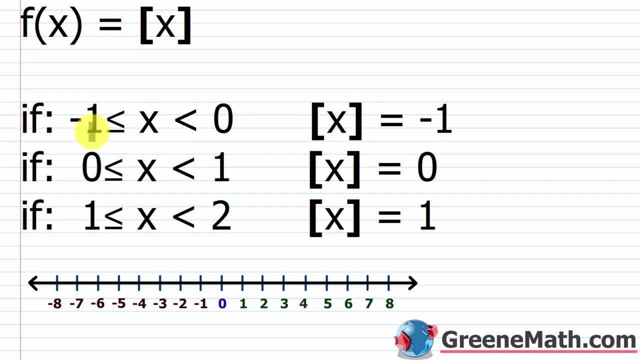 to the nearest integer. So in the case where you have f of x equals the greatest integer of x. if x is greater than or equal to negative one, but less than zero, what's going to happen is your value is going to be negative one. So let's say I'm on the number line and I'm somewhere like right here. Let's say I'm. 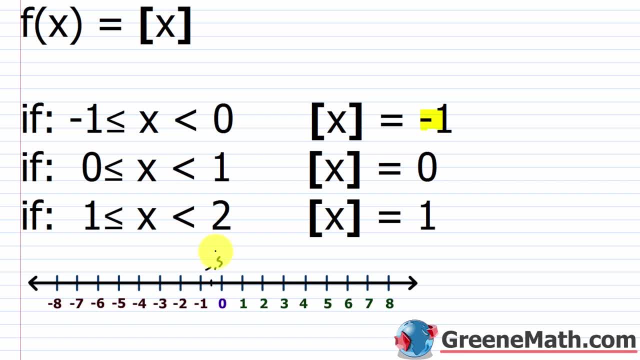 at negative 0.5.. If I round down to the nearest integer, I'm going to the left. So going to the left from that point puts me here. That's going to be the largest integer. that's less than or equal to negative 0.5.. So it's very, very tricky if you don't reread the definition over and over and 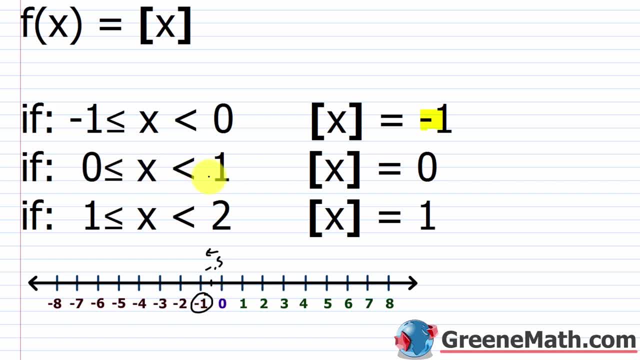 over again. If x is greater than or equal to zero, but less than one, so let's say it's 0.5. now, Well, if I round down, I'm going to get to zero. So in this case I'm at zero, and so on and so forth. 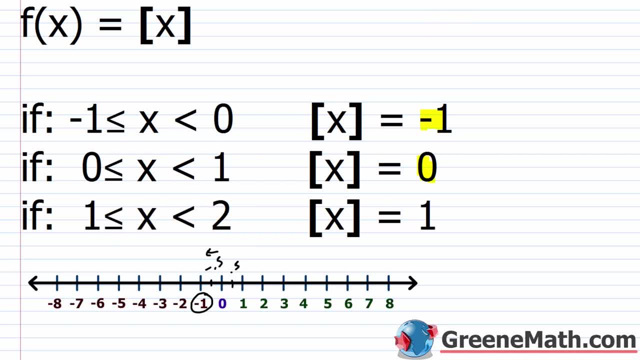 If x is greater than or equal to one and less than two. so let's say I was at 1.5.. Well then, I'm rounding down to one. So I'm always going to round down to negative 0.5.. So I'm going to round down to. 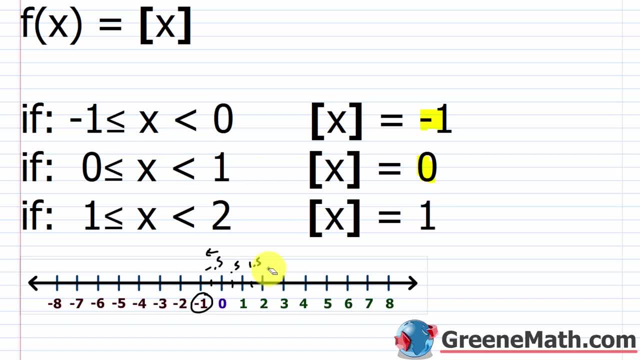 the nearest integer If I'm at an integer itself. so let's say I was at one. Let's say I plug that in. Well, it's just going to be the integer. It can be equal to that. But if I'm anything less, 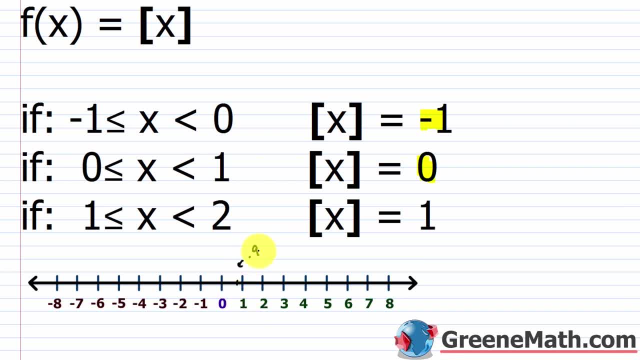 than one. let's say, I'm at, you know 0.9998.. Well, in that case I've got to round down to zero, right? I'm in this category where x is greater than or equal to zero, but less than one. If I'm. 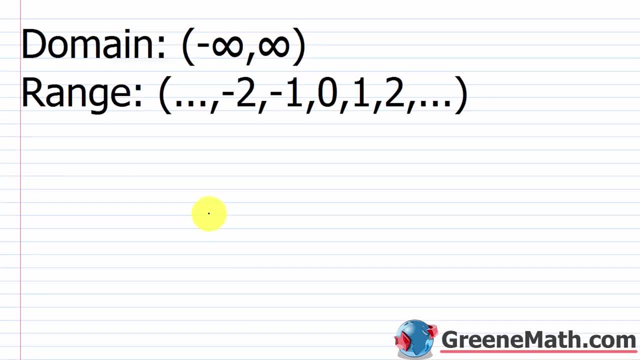 not at one exactly. I've got to round down, So I'm going to end up at zero. So for the domain and for the domain, I can plug anything I want in. for x There's no restrictions, right, All real numbers. But for my range, remember, if I plug something in here the output is going to be the 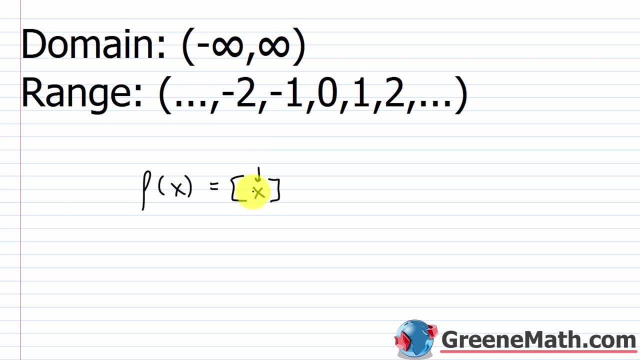 largest integer that's less than or equal to the value I plugged in. So I'm limited to just getting integers back. So my range will be the set of integers. So we sometimes refer to the greatest integer function as a step function because of the shape of the graph And the way it looks. 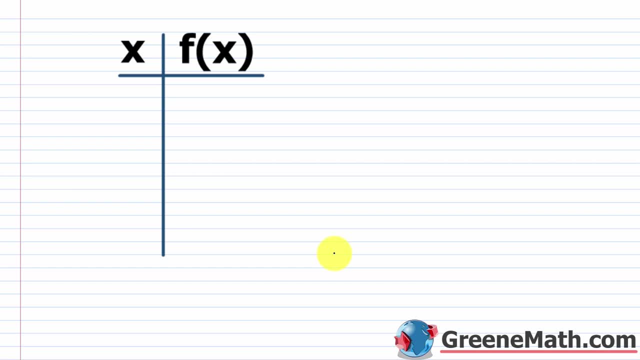 kind of like. that is because for a range of x values you now have the same y value. So for an x value that is greater than or equal to negative three, but less than negative two, we know y would be equal to negative three If x was greater than or equal to negative two, but less than negative. 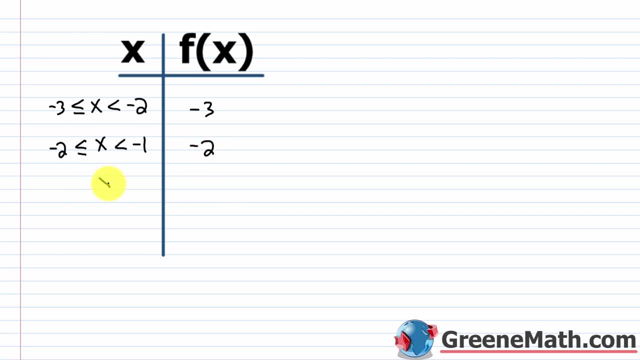 one, we know y would be negative. two, If x was greater than or equal to negative one, but less than one, we know y would be zero. You know. so on and so forth. You'll see the pattern in a minute. 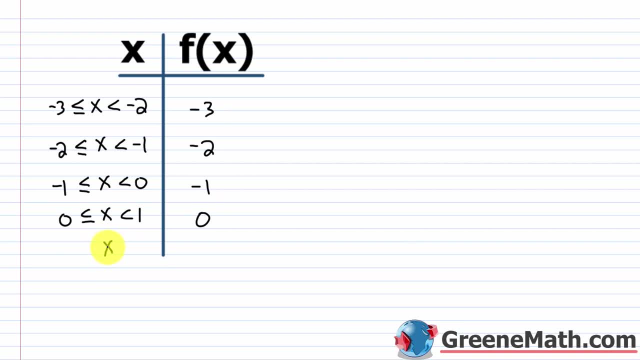 Let me do one more of these, and then you'll be able to draw as many as you want. So if x was greater than or equal to one but less than two, y would be one. So let's just think about this on. 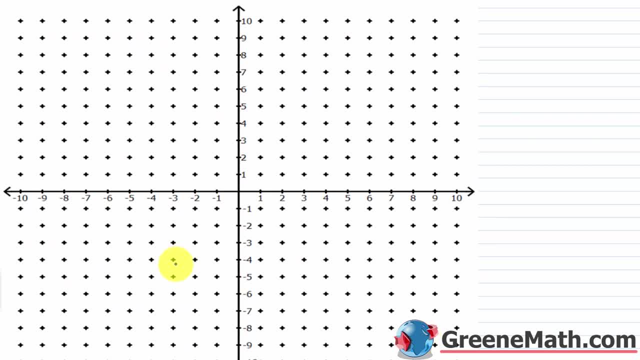 the coordinate plane here. So again, if x was greater than or equal to negative three, but less than negative two, y would be negative three. So let's find a y value of negative three. Let's go x value of negative three. I put a bracket here to say this is included here. Then I'm going to 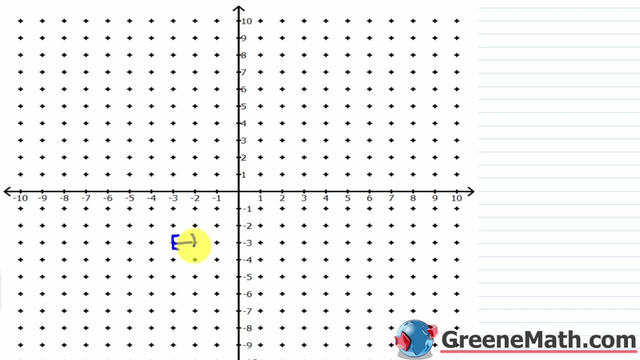 draw a horizontal line across. Then at negative two I'll put a parenthesis to say it's not included. Then I'm just going to step up to the next integer for x and I'm going to do the same thing. I'm going to put a bracket to say negative two is included. I'm going to draw a horizontal. 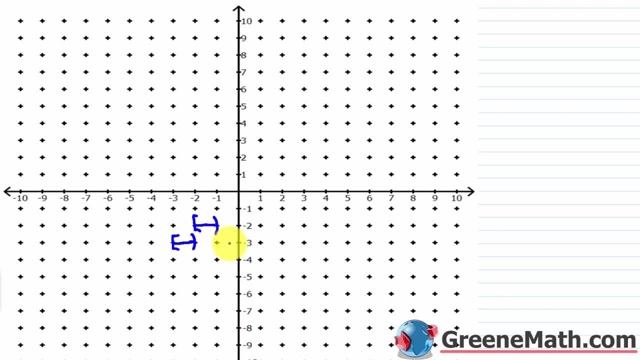 line to negative one. Negative one's not included. I'm going to step up again. put a bracket here. go over to the next integer. put a parenthesis. Step up again. bracket parenthesis. Step up again. bracket parenthesis. Step up again. 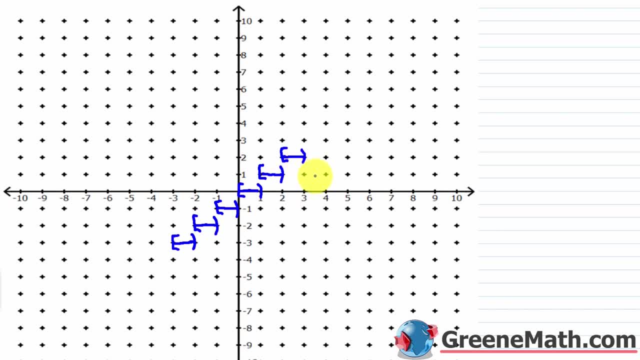 bracket parenthesis, Step up again. So again, for a given range of x values there's a set y value. So if x is between negative three and negative two, where negative three is included, y is negative three. If x is between negative two and negative one, negative two. 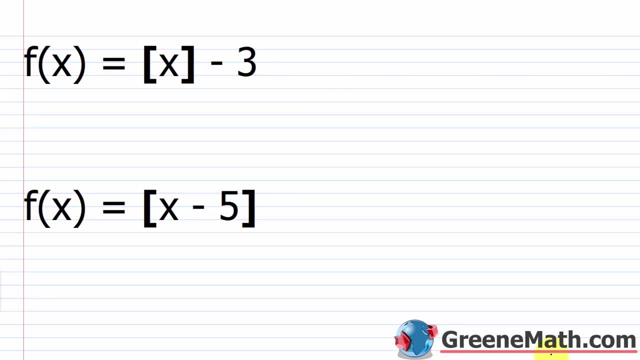 exceeds y, James Hebrews. So we're doing the same thing now, and if y is negative two, I'm going toY going to quit on it. Then I'm just going to consider what x equals on the next added valueلا s. 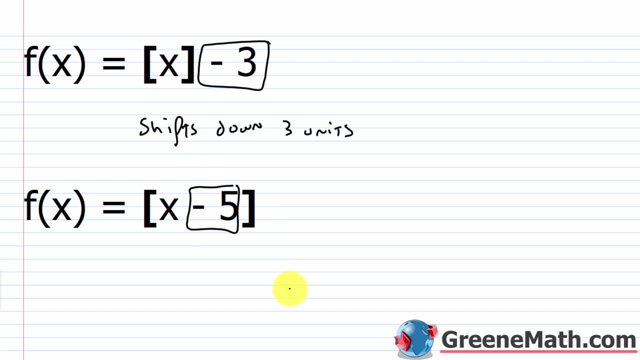 minus 5 in for x, and this is what I get. So this is going to shift to the right by 5 units. So this shifts right by 5 units. Hello and welcome to Algebra 2, Lesson 75. In this lesson, 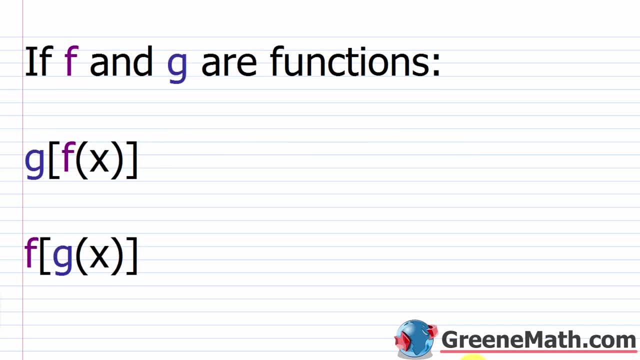 we're going to learn about the composition of functions. So at some point in your Algebra 2 course- or this might even happen to you in an Algebra 1 course- you're going to come across this topic known as function composition or again you could say, the composition of functions. 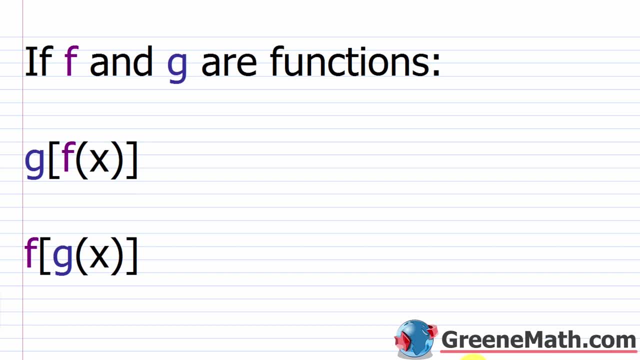 So what this really involves is some heavy substituting and some simplifying. It's a very, very easy topic once you understand the notation that you're going to be working with. So the first thing you're probably going to see in your textbook: if f and g are functions, this is read: 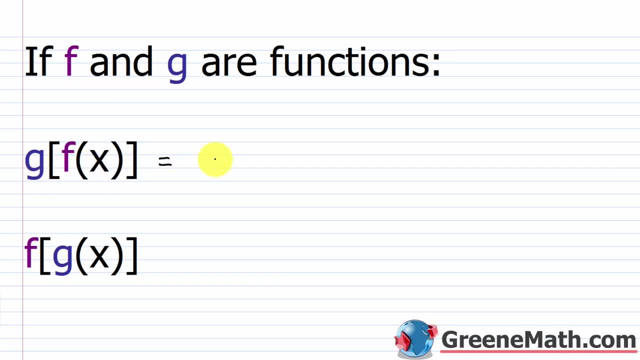 g of f of x. and you could also write this like this: You could say g of f of x. and then another way to write it, a way that you've probably never seen before: you'll have g of f of x. This way, right here, is the way that confuses most students. 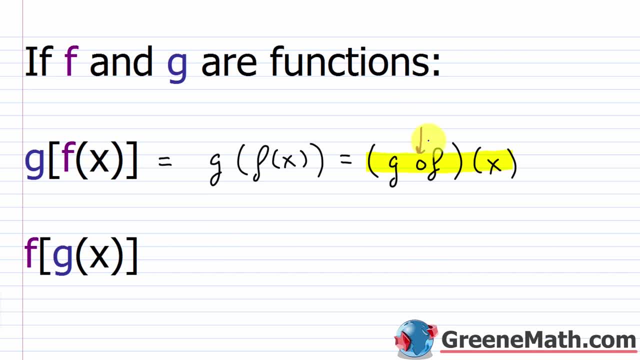 It's a foreign notation. People always look at that and think it's a multiplication symbol. It's not. You can see that it's not filled in. This is not g multiplied by f in any way, shape or form. So this is g composed with f. okay, That's what this is basically. 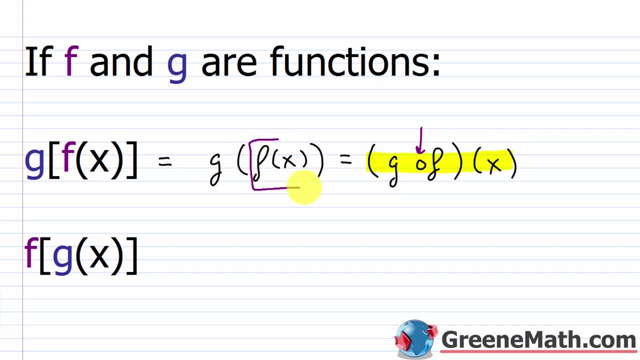 but it's just a fancy way of saying: hey, I'm going to take f of x and I'm going to plug it in for x in g of x. We'll see that when we get to the examples in a second. Then this guy right here: 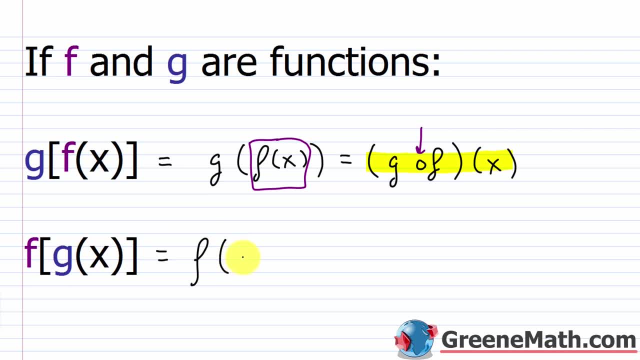 we've kind of flipped the order around. So here this is f of g of x, and we could also write this like this: We could say f of g of x. Essentially, all I'm doing here is I'm taking g of x. 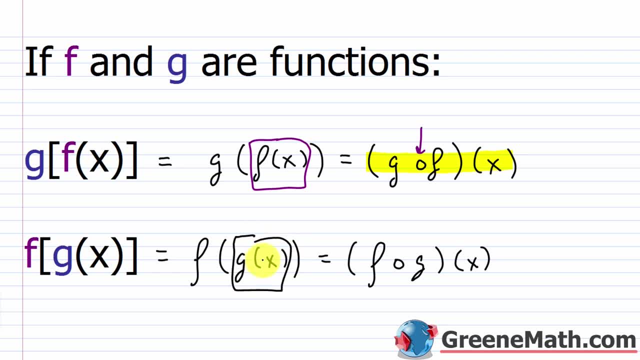 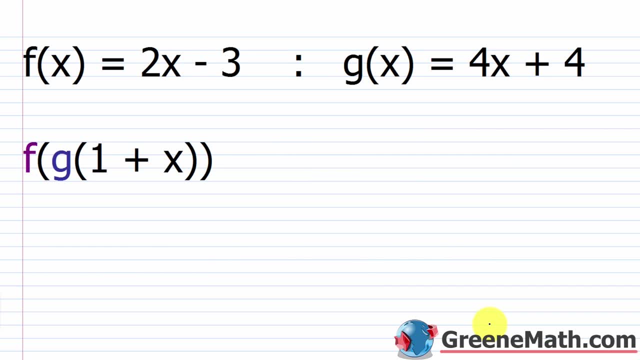 and I'm plugging it in for x in the function f of x. So this section is all going to be about just substituting and simplifying. So before we kind of jump in and look at the first example, I want to make sure you understand the most basic. 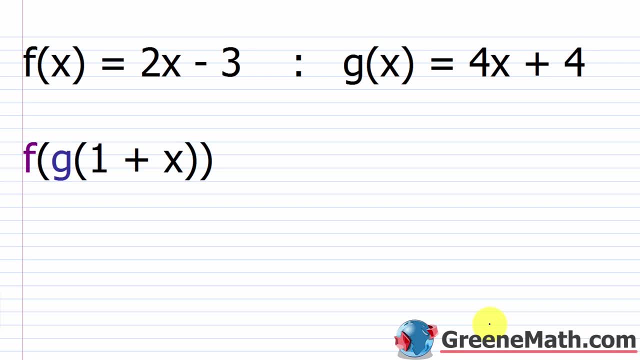 thing when it comes to function notation. If I take this f of x here, and in this case it's 2x minus 3.. So that's our function. If I ask you, what is f of 2?? What am I asking for? 2 is in the. 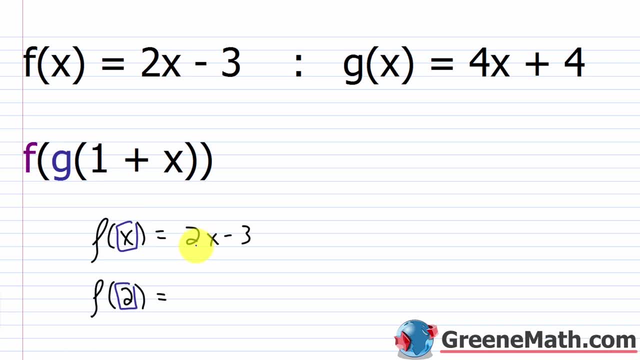 x. So what I'm asking for is: what is the function's value when I plug in a 2 for x? All I'm asking for So this is: 2 multiplied by plug in a 2 for x, then minus 3.. 2 times 2 is: 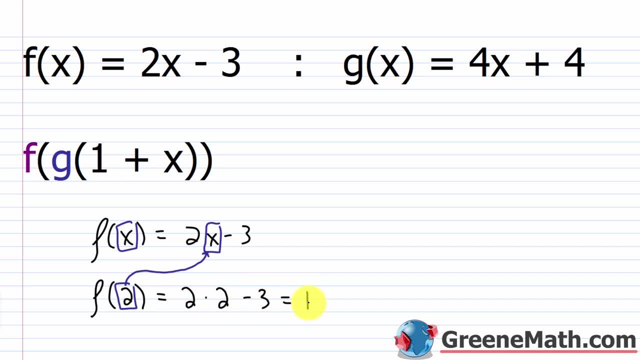 obviously 4.. 4 minus 3 is 1.. So f of 2, or the function's value when the independent variable x is 2, is 1.. So you can say f of 2 is 1.. Now I'm not limited to just plugging in numbers. 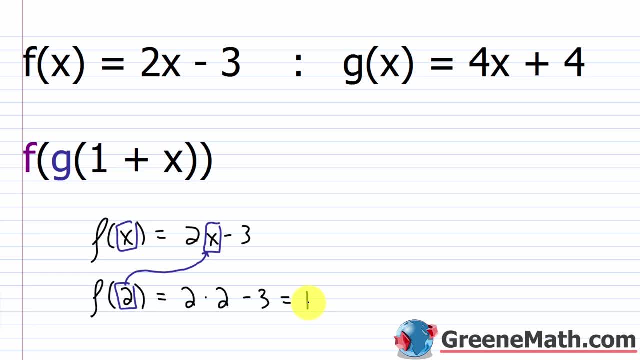 for my variable. I can take something more complex and plug it in. So what if I said I want f of I don't know? let's say x minus 1.. Well, all I'm going to do is I'm going to plug in an x minus. 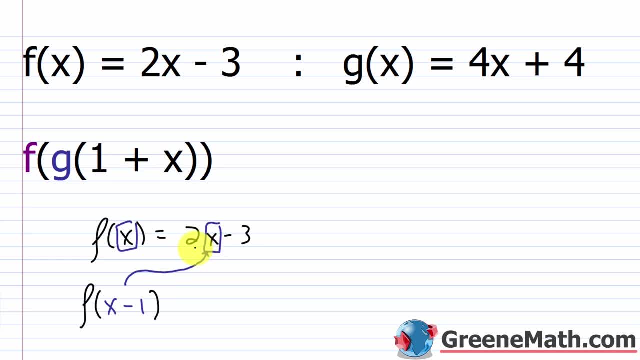 1 for x and I'm going to evaluate. So in this case I would have 2 multiplied by for x. I'm plugging in an x minus 1.. So I'm going to use parentheses. So x minus 1, that quantity then. 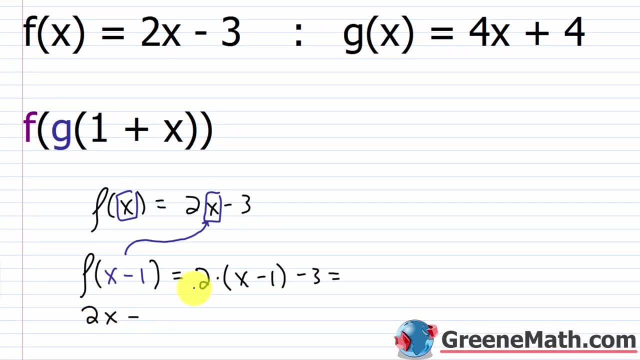 my distributive property: 2 times x is 2x, then minus 2 times 1 is 2,, then minus 3.. You have 2x which you can't do anything with. Negative 2 minus 3 is minus 5.. So f of x minus 1 is equal to 2x. 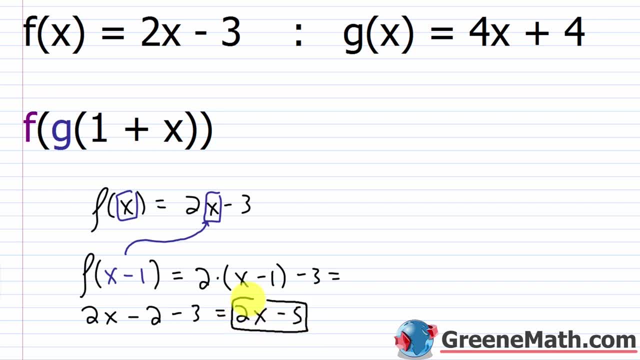 minus 5.. Now, I didn't get a numerical value there, but I still found what the function would be if I plugged in an x minus 1 for the independent variable x. That's all I'm asking for. So that's all we're really going to be doing here. We're just plugging things in and simplifying. 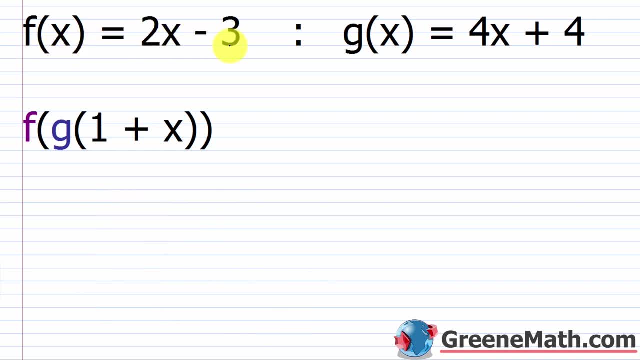 So, for the first example, we're given f of x, which equals 2x minus 3, and we're given g of x, which is equal to 4x plus 4.. What we want to find is f of g of 1 plus x. Now, if I saw g of 1 plus x. 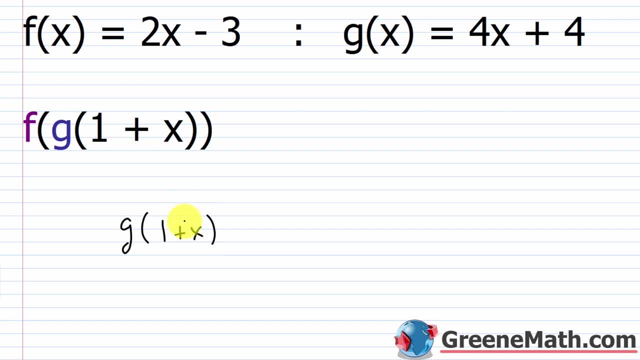 what would that mean? It would mean that I'm taking a 1 plus x and I'm plugging it in for x, function g of x. So you would start by finding this part first, because, whatever this is, that's what I'm plugging in for x in f of x. So you're starting on the inside and you're working. 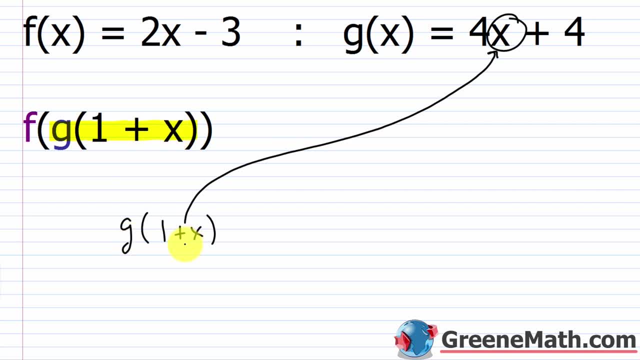 your way out. So let's find g of 1 plus x, or you could flip that around and say this is g of x plus 1, whatever you want to do. So this equals 4 multiplied by. again I'm plugging in for x there. 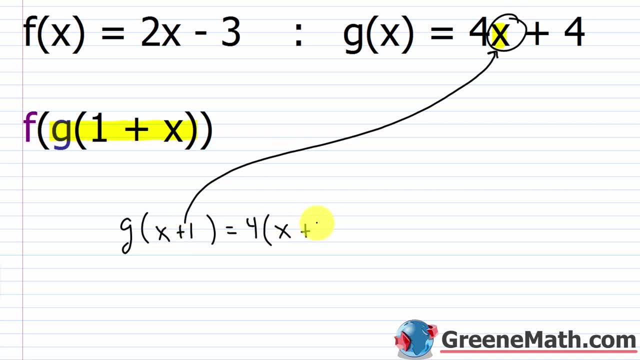 What am I plugging in? I'm plugging in an x plus 1.. So x plus 1,, and then plus 4.. So 4 times x is 4x, then plus 4 times 1 is 4,, then plus 4.. So this gives me what. 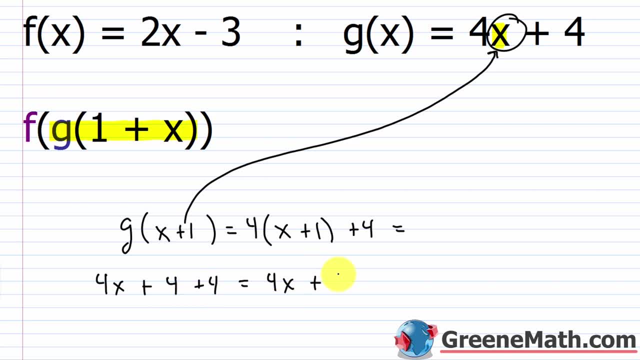 4x, can't do anything with that. then plus 4 plus 4 is 8.. So I get 4x plus 8 as the result there. So now let's go back up here. I'm just going to write that g of x plus 1 is equal to 4x plus 8.. 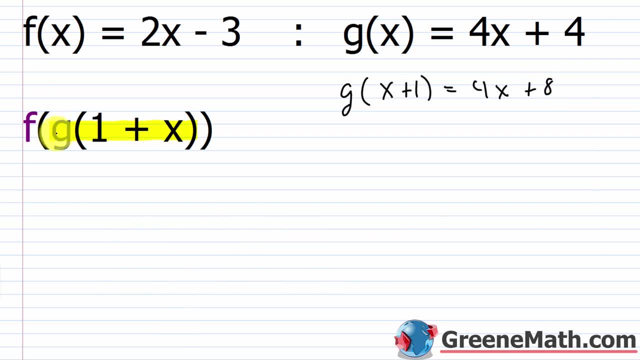 And I can erase this. So now that I know that g of 1 plus x or g of x plus 1, however you want to say, that is 4x plus 8, I can really say that this problem is: f of this right here is 4x plus 8.. So f. 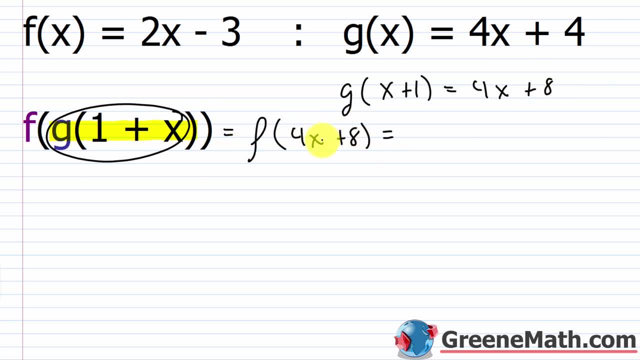 of 4x plus 8.. And then I can just plug a 4x plus 8 in for x in this guy right here. So this would be what It would be: 2 multiplied by the quantity 4x plus 8.. 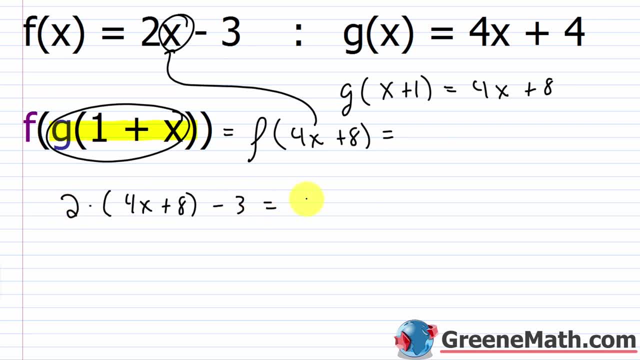 And then minus 3.. So 2 times 4x is 8x, And then 2 times 8 is 16.. So plus 16. And then minus 3.. So 8x. there's nothing I can do with that. 16 minus 3 is obviously 13.. So you get 8x plus 13. 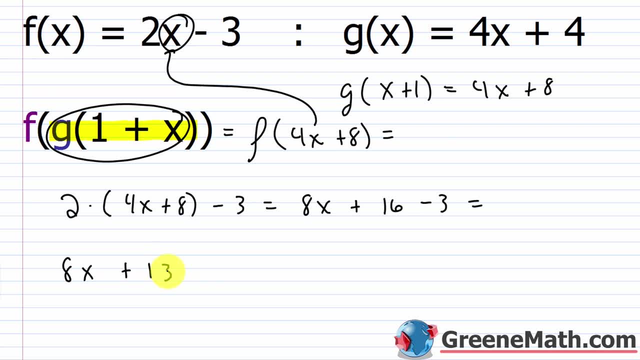 as your answer. So the result here, f of g of 1 plus x- is equal to 8x plus 13.. So nothing really super complicated here. It's just a lot of substituting and simplifying. All right, let's take a look at another example. 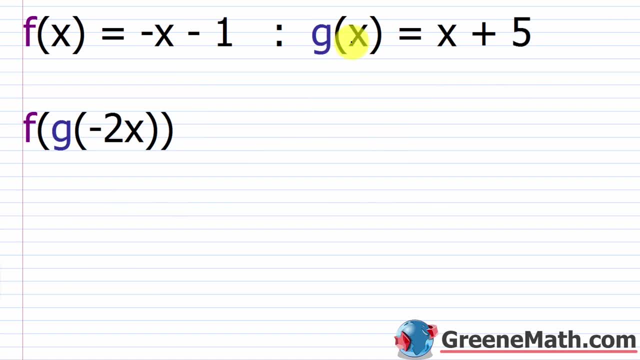 So we have f of x equals negative x minus 1.. We have g of x equals x plus 5.. And we want to find f of g of negative 2x. So again, I'm going to start out with this guy right here: What is g? 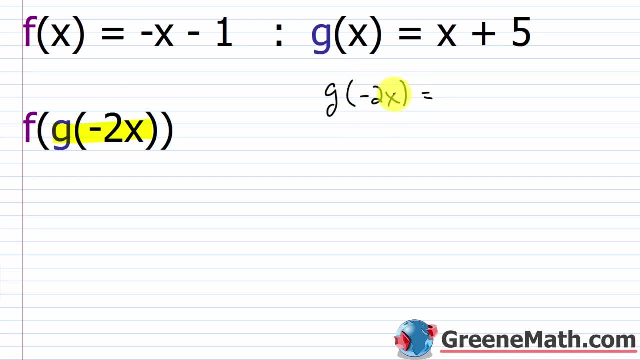 of negative 2x. Well, again, all I'm going to do is plug a negative 2x in for x in g of x. So this would be what I'm going to plug in a negative 2x there. So it would just be negative 2x and then plus 5.. 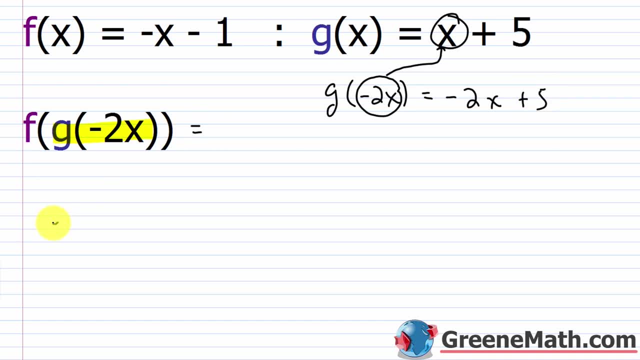 Super, super simple. So now all this would be is f of. I know that this part right here is this, So f of negative 2x plus 5 would give me what Well, I'm plugging this in for this right here. 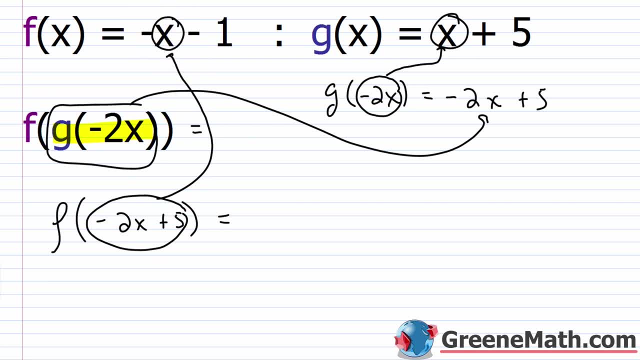 Be careful of that negative out in front. You want to account for that. So I'm going to have a negative times the quantity. So I'm going to plug in a negative 2x plus 5. And then I'm going to plug. 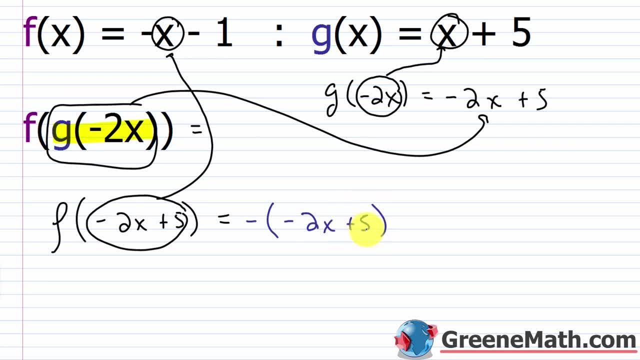 in a negative: 2x plus 5.. That's what I'm plugging in for: x right there And then minus 1.. So I'm going to distribute that negative to each term. So in other words, you can think about this as a. 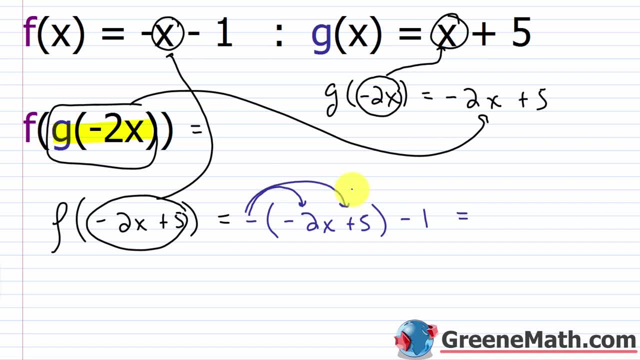 negative 1, multiplying each term. You're just going to change the sign. So instead of negative 2x, I'll have 2x. Instead of positive 5, I'll have minus 5.. And then I'll have minus 1.. So you'll. 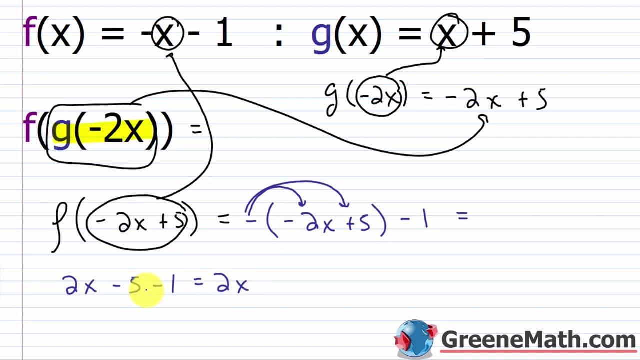 have 2x. You can just say negative 5 minus 1 is negative 6. So this ends up being 2x minus 6.. So f of g of negative 2x ends up being 2x minus 6.. All right, for the next one we'll look at g of x. 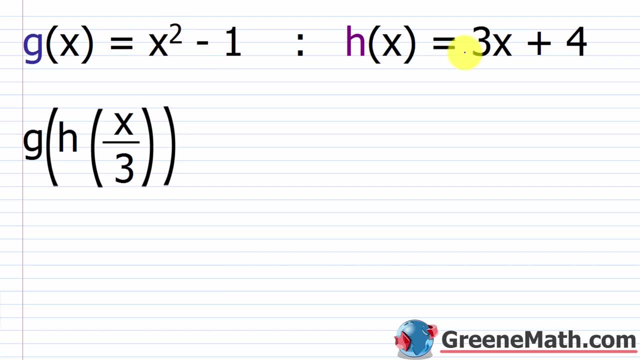 which equals x squared minus 1, and h of x, which equals 3x plus 4.. We're trying to find g of h of x over 3.. All right, so again I want to start with the inside right here. So we want to find: 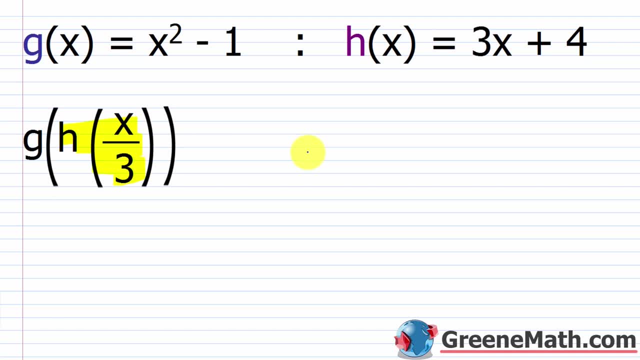 h of x over 3.. So what is that going to be? Well, here's h of x. So we want h of x over 3.. So this equals- I'm just going to plug this in for x in my function- So we'd have 3 multiplied by 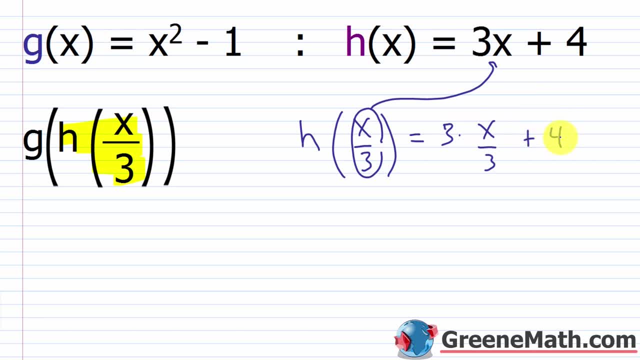 x over 3, then plus 4.. What's going to happen is this will cancel with this and I'm left with x, So this ends up being x plus 4.. So this part right here is nothing more than x plus 4.. 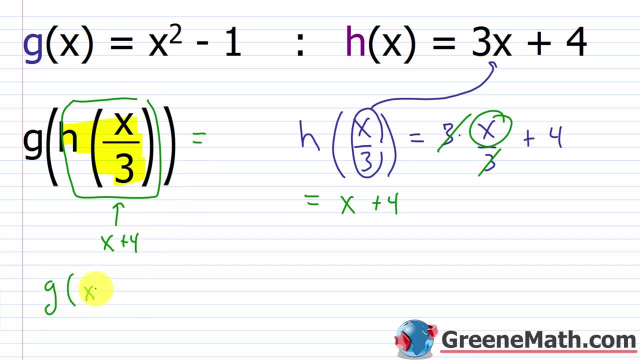 So this would be equal to g of x plus 4, and that would be what I'm taking: x plus 4, that quantity and I'm plugging it in for x in g of x, So I would have the quantity x plus 4,. 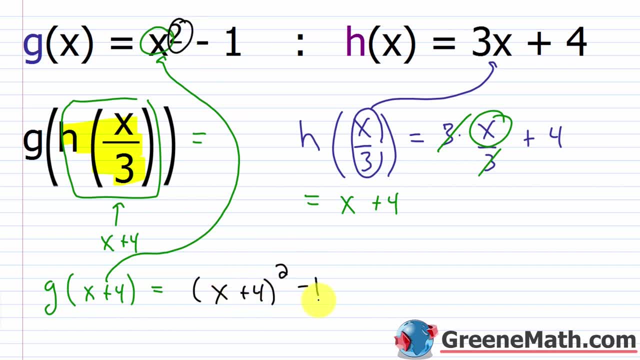 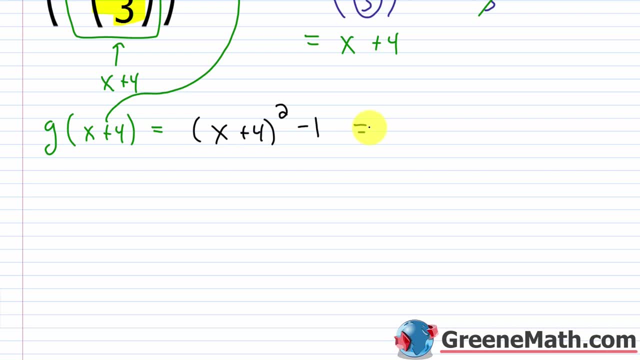 that would be squared, and then I'm subtracting away 1.. So I'm going to use my special products formula. there I can square x plus 4, that quantity pretty quickly. This would be x squared plus 2 times x squared. So I'm going to use my special products formula. there I can square x. 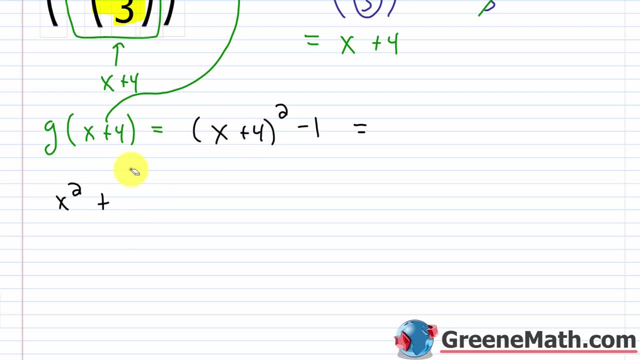 times 4.. 2 times 4 is 8.. 8 times x is 8x. So this would be plus 8x. And then, lastly, plus 4, squared is 16, and then minus 1.. So you'd have x squared plus 8x. 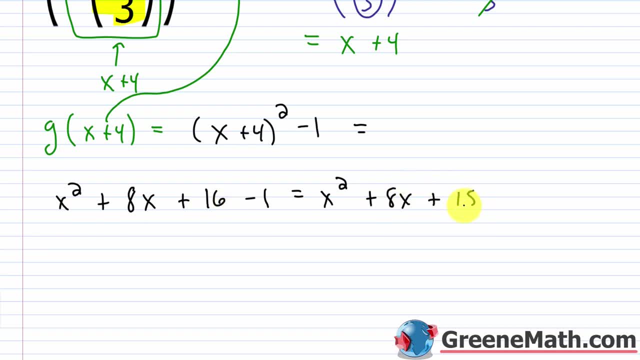 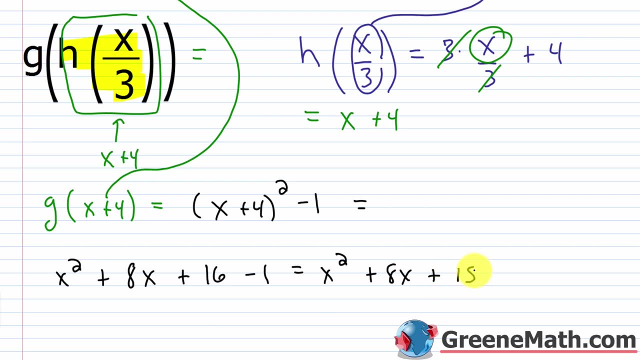 and then 16 minus 1 is 15.. So plus 15.. So we can say: g of h of x over 3 is equal to x squared plus 8x plus 15.. All right, let's take a look at another one. So we have g of x is equal to: 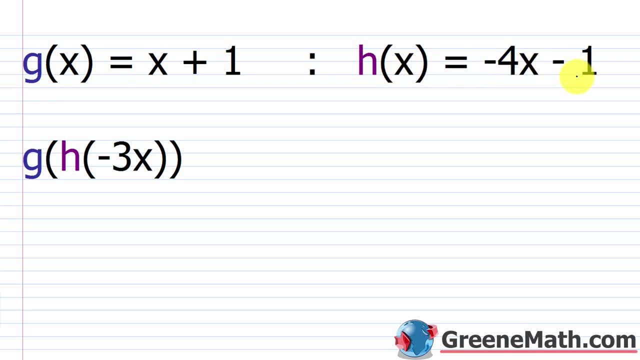 x plus 1, h of x is equal to negative 4x minus 1.. So we want g of h of negative 3x. So all I want to do is start out by finding h of negative 3x, So h of negative 3x. just plug a negative 3x in. 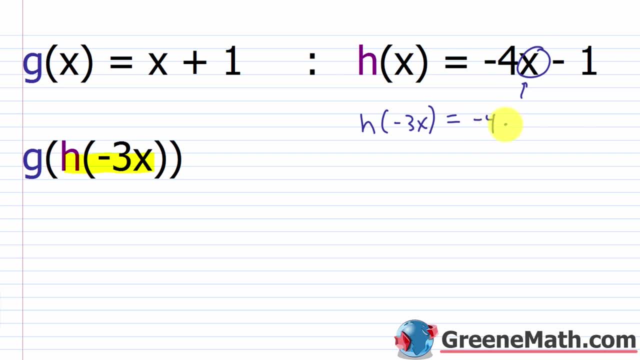 for x here. What would that give me? You'd have negative 4 multiplied by negative 3x. plug it in for x there, then minus 1.. Negative 4 times negative 3 is 12.. So you'd have 12x and then minus 1.. So this guy right here. 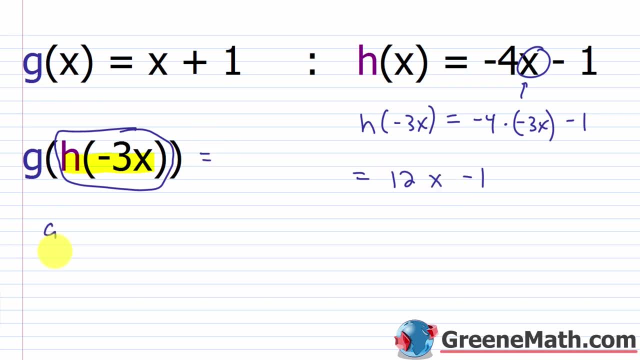 is 12x minus 1.. So this would become g of 12x minus 1, which equals what Plug in a 12x minus 1 there? So you would have 12x minus 1, then plus 1.. Pretty simple Negative. 1 plus 1 is 0. 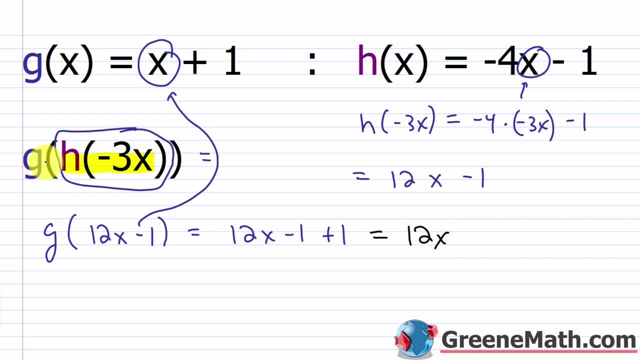 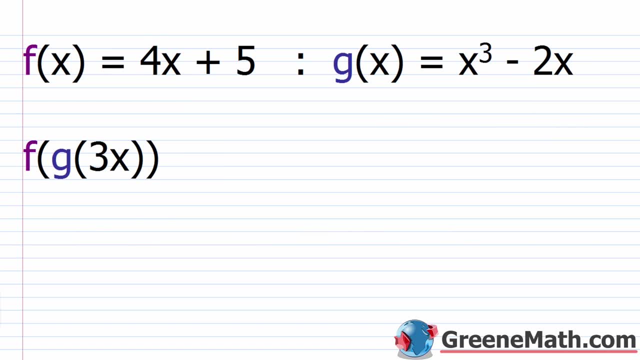 So this just turns into 12x. So g of h of negative 3x is just 12x. All right, what about f of x equals 4x plus 5, and then g of x equals x cubed minus 2x. So here we want f of g of 3x. So I start with g of 3x. So 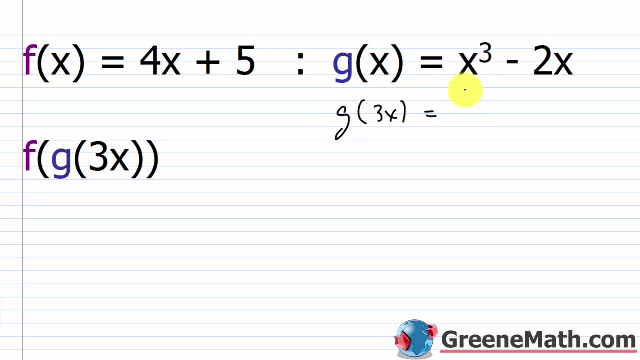 g of 3x. this would be what Plug in a 3x there. So you'd have 3x cubed minus 2 times plug in a 3x there as well. And what does that give me? 3x cubed would be what? 3 cubed is 27,. right, 3 times 3 is 9,. 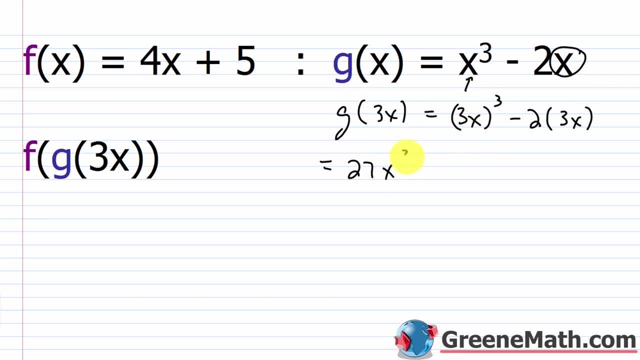 9 times 3 is 27.. So 27,, and then x cubed and then minus 2 times 3 is 6.. 6 times x is 6x. So you get 27x cubed minus 6x. And I want to take this guy and I want to plug it in for x here. 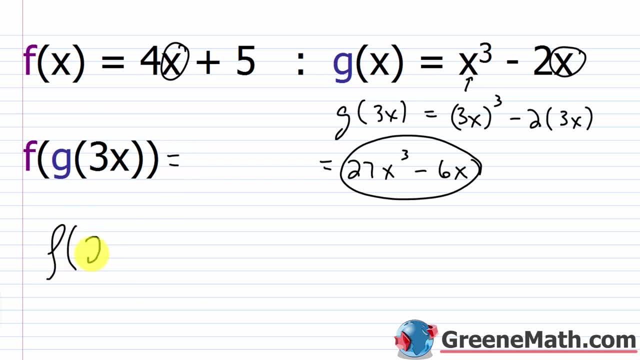 So, in other words, I want to say that I have f of 27x cubed minus 6x, and this would give me what It would give me: 4 multiplied by 27x cubed minus 6x Again. 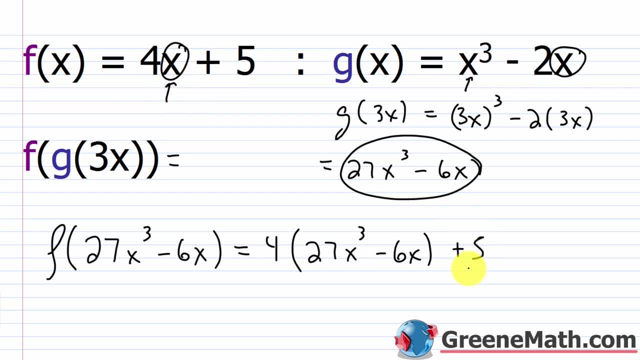 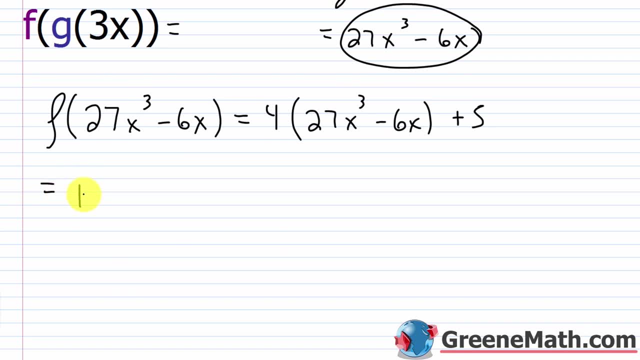 just plugging this in for x there, Then you have plus 5.. All right, so what does this give us? We would have 4 times 27,, which is 108, then times x. cubed, then minus 4 times 6 is 24,. 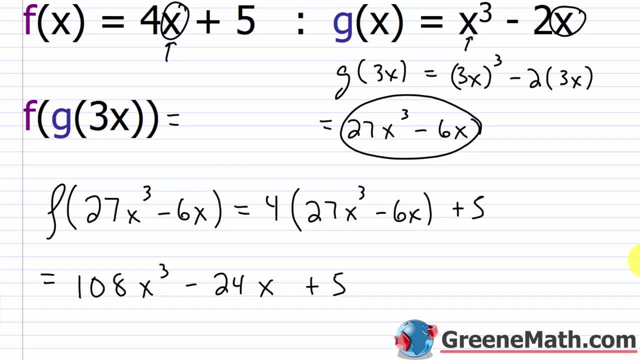 and times x, then plus 5.. So we can say f of g of 3x, 3x is equal to 108x cubed minus 24x plus 5.. All right, let's take a look at another one. 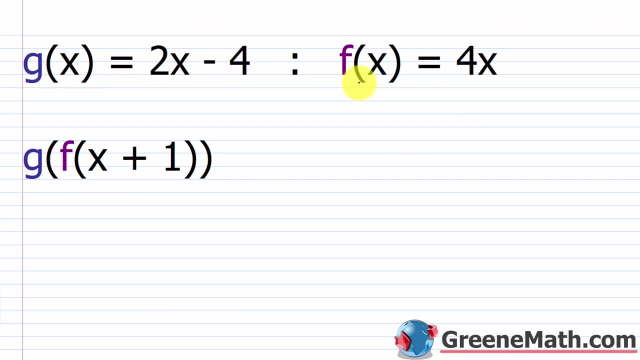 So we have g of x equals 2x minus 4.. We have f of x equals 4x, So we want g of f of x plus 1.. So if I had f of x plus 1, this part right here, what would that give me? This is 4 multiplied by. 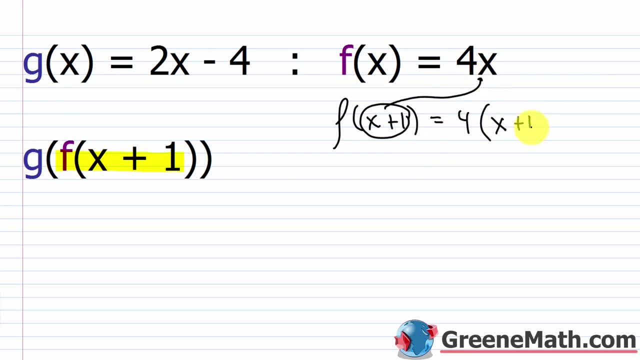 this gets plugged in for x, So 4 times the quantity x plus 1, this gives me 4x plus 4.. So that's what's going right here. So in other words, this is g of 4x plus 4.. So this would be equal to- I have a 2 multiplied by. 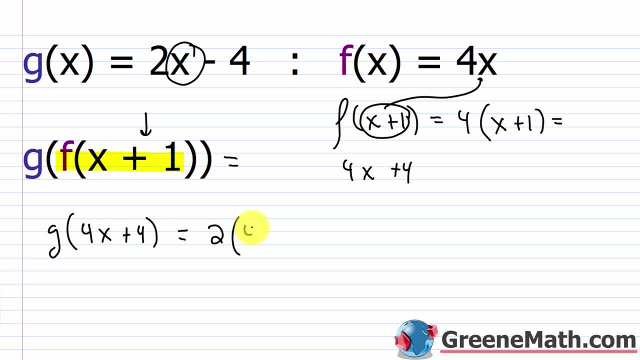 plug in a 4x plus 4 in for x, So 2 times the quantity 4x plus 4, and then you have minus 4.. Use the distributive property: 2 times 4x is 8x, then plus 2 times 4 is 8,. 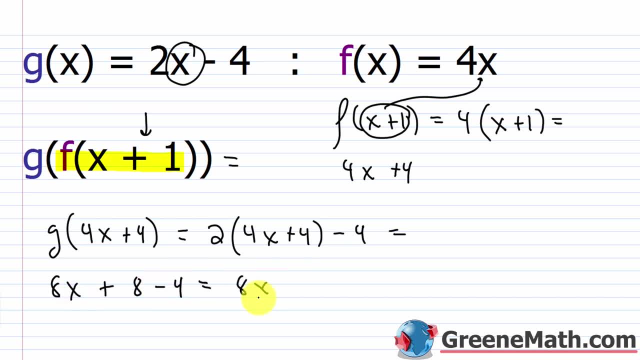 then minus 4.. So you'd have 8x. 8 minus 4 is 4, so 8x plus 4.. So g of f of x plus 1 gives us 8x plus 4.. Let's take a look at one more. Again, it's a very easy concept, as you can see. 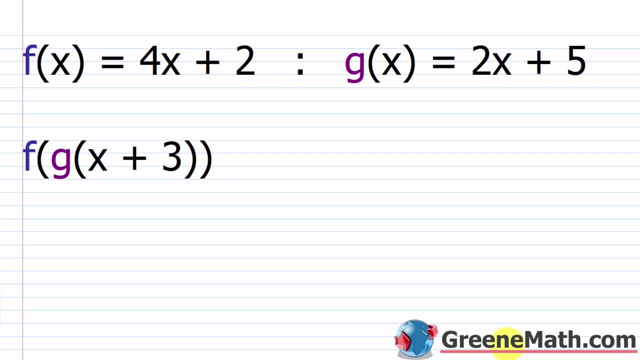 You're just taking one function and you're using it as an input in another function. So we have f of x equals 4x plus 2.. We have g of x equals 2x plus 5.. So what is f of g? 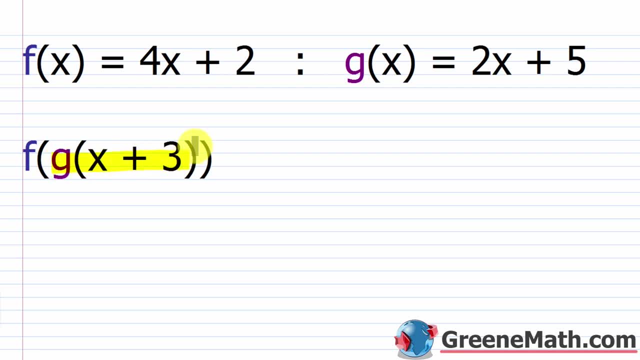 of x plus 3?. So again, I start out with g of x plus 3.. So g of x plus 3 gives me 1. This would be 2 times this quantity, right? I'm plugging that in for x. 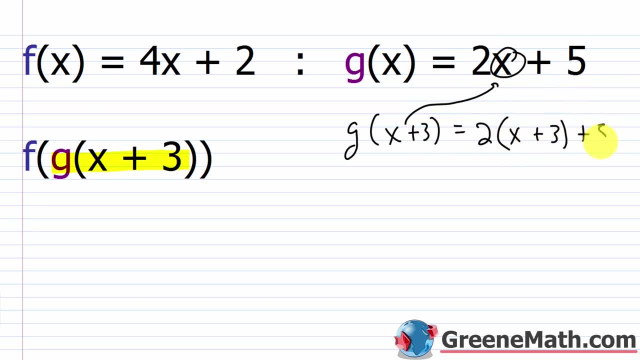 So 2 times the quantity x plus 3, and then plus 5.. 2 times x would be 2x plus 2 times 3 is 6, plus 5.. So this gives me 2x plus 6 plus 5 is 11.. So that's this part right here. So in other words, 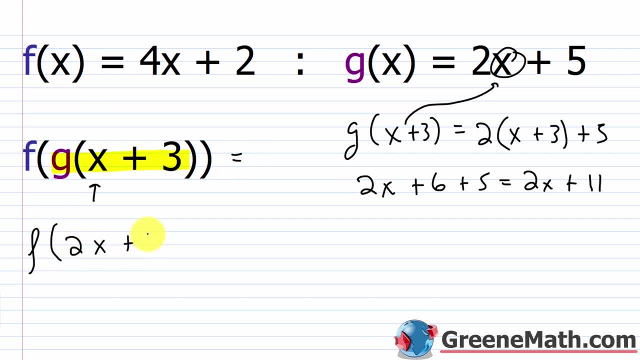 you would have f of 2x plus 11.. So this gives me what You would have 4 times. in place of x I'm plugging in a 2x plus 11.. So 4 times the quantity 2x plus 11, and then plus 2.. 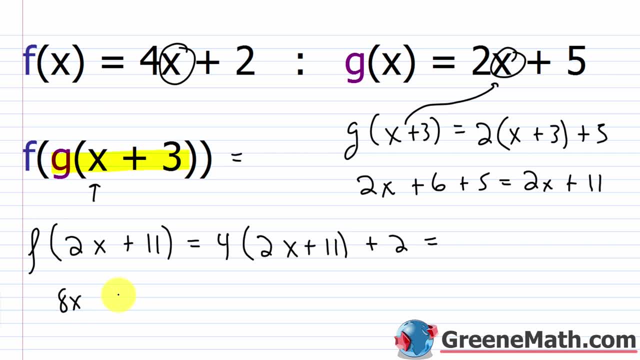 So use my distributive property: 4 times 2x is 8x, and then plus 4 times 11 is 44, and then you have plus 2.. 8x would stay the same. nothing I can do with that. 44 plus 2 is just 4x. 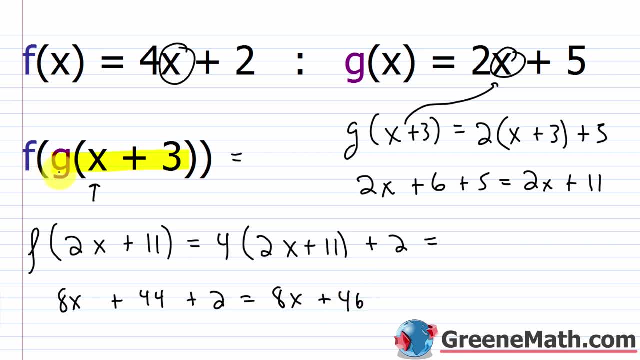 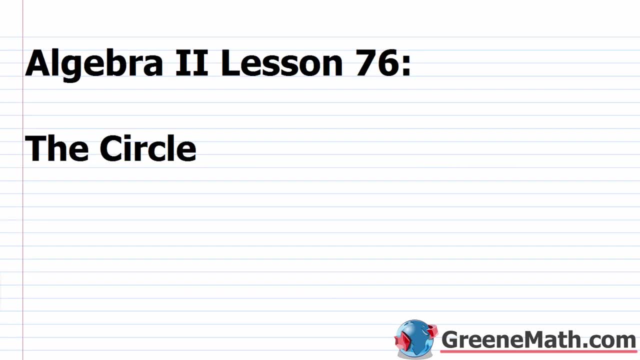 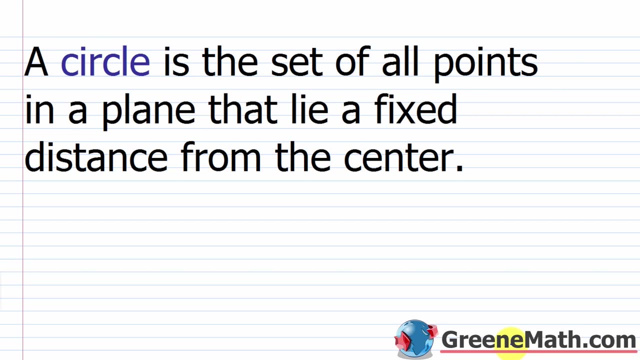 46. So we end up with f of g of x plus 3 has 8x plus 46.. Hello and welcome to Algebra 2, Lesson 76. In this lesson we're going to learn about the circle. So at some point in your Algebra 2 course you will begin talking about conic sections. 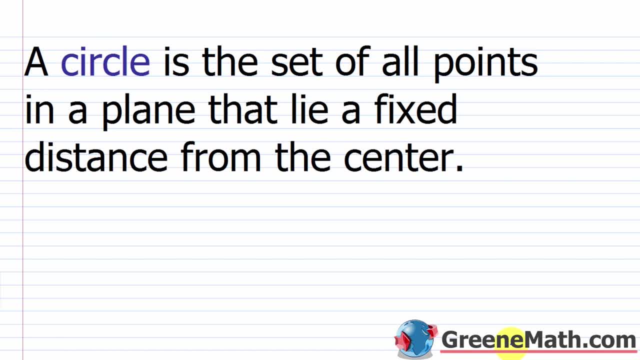 So these include parabolas, circles, ellipses and hyperbolas. Now, we already discussed how to work with parabolas before. Now we're just going to tackle the subject of circles. So the first thing is: let's just get a. 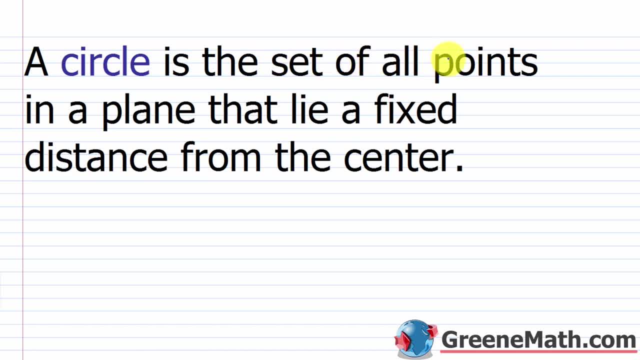 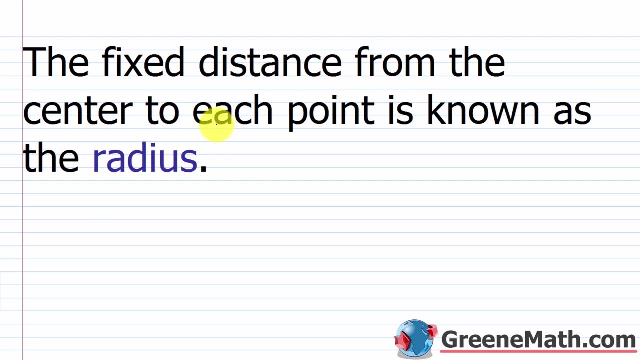 brief definition. going So, a circle is the set of all points in a plane that lie a fixed distance from the center. So the next part of that is to say that the fixed distance from the center to each point is known as the radius. This is something you want to write down. 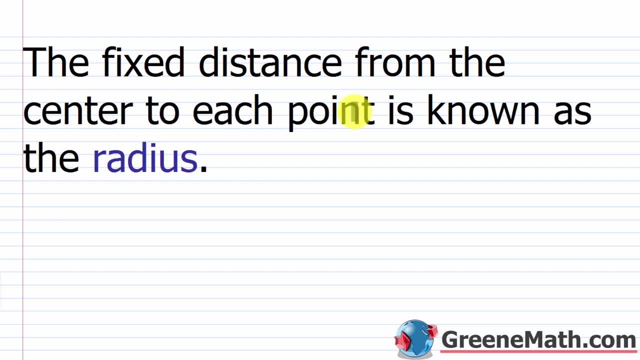 because we're going to use it in a minute when we talk about the distance formula. So the fixed distance from the center, so from the center to each point on that circle, is again known as the radius. Now, the first thing you're going to come across when you get into the topic of 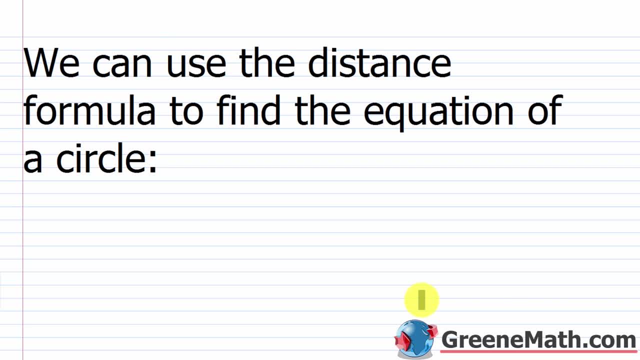 circles is going to be the equation of the circle. Now this is given to you in standard form, otherwise known as center radius form, And it allows you to look at the equation and very clearly define the через equation. you're going to need to find the equation of the circle. 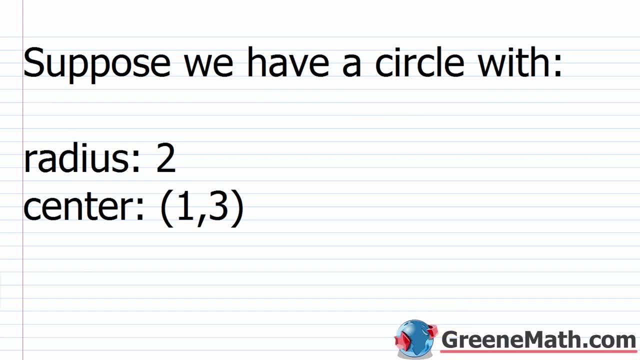 So how do we go about doing that? Let's think about what the distance formula does for just a second. I want you to remember that the distance formula allows us to take two points on a coordinate plane and find the distance between them. So if I have two generic points, let's just say x sub one, y sub one. 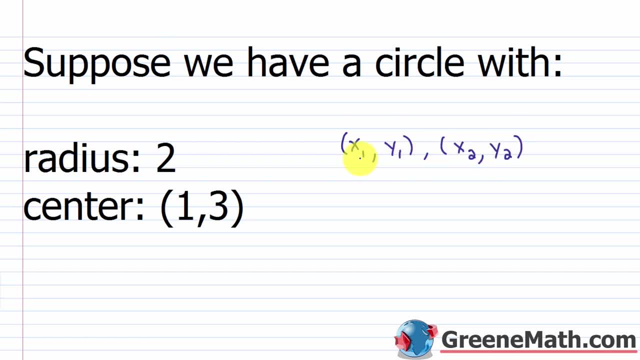 and x sub two, y sub two. Okay, these could be any two points in a line, but what I'm going to do is I'm going to divide all these by the space between them, be any two points. Well, the distance between them is given by this formula: The d or the. 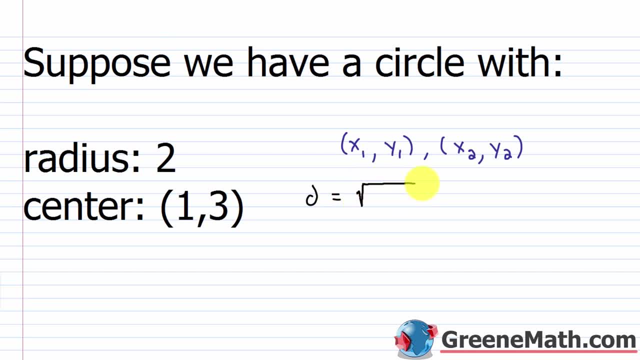 distance equals, we would have the square root of you have x sub 2 minus x sub 1, this quantity squared. then, plus, you'd have y sub 2 minus y sub 1, this quantity squared. Now how do we use this information to obtain the equation for a circle? Well, if I'm given 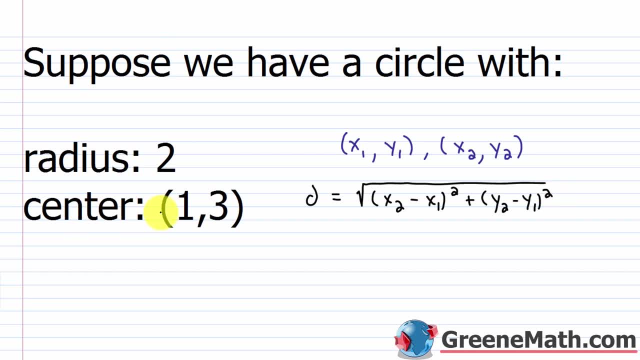 the center of the circle, which is not actually on the circle. it's in the center and I'm given the radius. what I can say is that the radius gives me a distance from the center to any point on that circle. So generically I could say that the distance is 2. The distance: 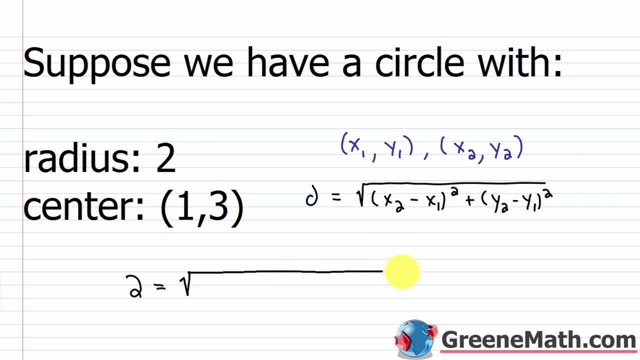 is 2, and this equals the square root of. so let me just replace this point right here, this x sub 1 and y sub 1, with a known point of 1, comma 3.. And let's plot, Let's log into the distance formula, So the distance between any point, instead of calling. 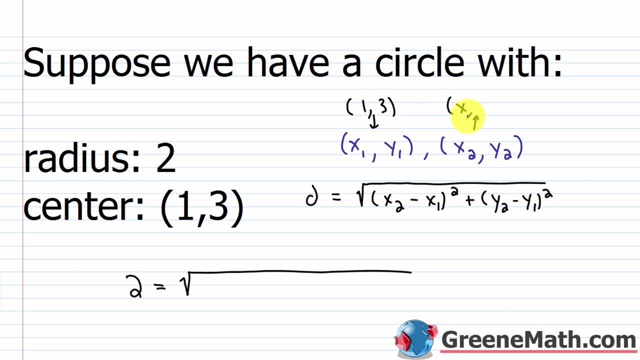 it x sub 2, y sub 2, I'm going to call it x comma y, So any x comma y point that you come up with, because again we know that the distance between them would be equal to 2, because our radius is 2.. So, following this, x sub 2 minus x sub 1, squared So x. 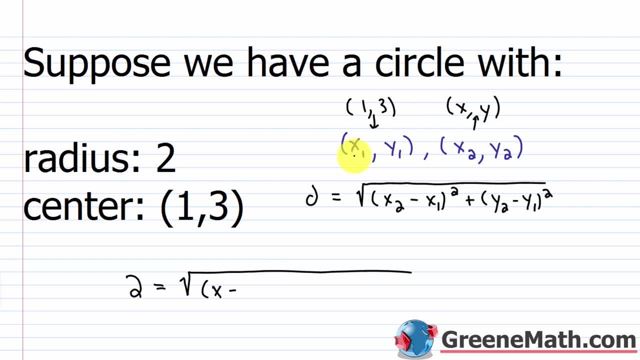 sub 2. now here I've replaced with x, so I would say x minus, where x sub 1 I replaced with 1.. So x minus 1, that quantity squared, then plus we would have y sub 2, which now I replaced. 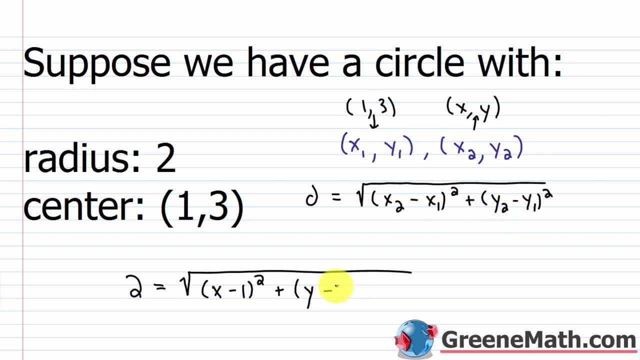 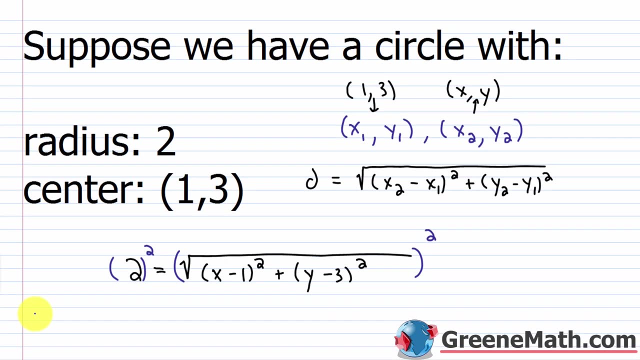 with y minus y sub 1, I replaced that with 3.. So then, this is squared. So so far, it's not actually where we need it to be. We need to do one additional step, which is to square both sides. So if I square both sides, 2 squared is 4, and this equals. 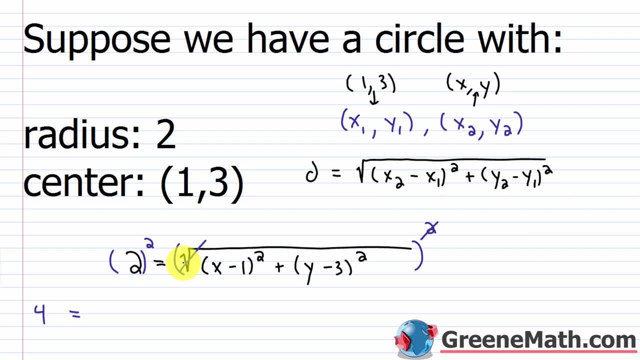 this cancels with this, So I'm just left with what is Underneath the square root symbol, which is the quantity x minus 1 squared plus the quantity y minus 3 squared. Now, for the purposes of what you normally see, I'm just going to. 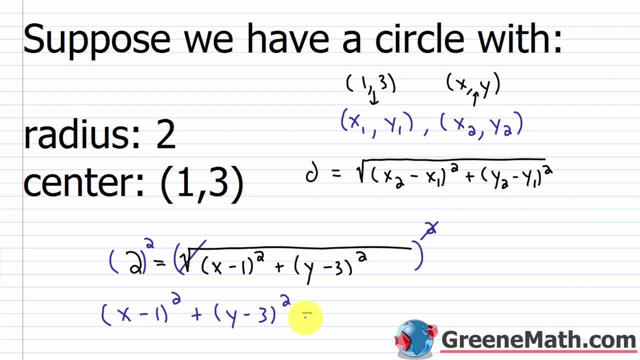 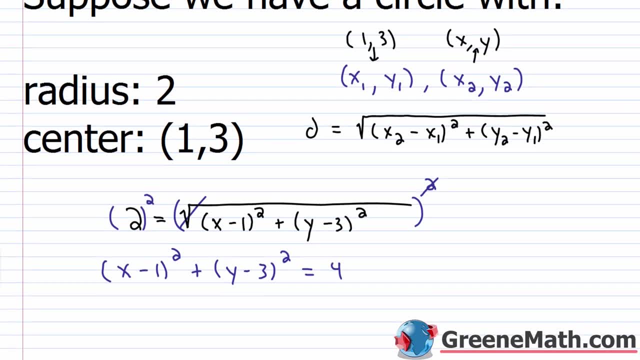 take this 4 that's over here on the left. I'm going to put equals 4 over here on the right, because this is how you're normally shown this equation. So this is your center radius form. This is your center radius. 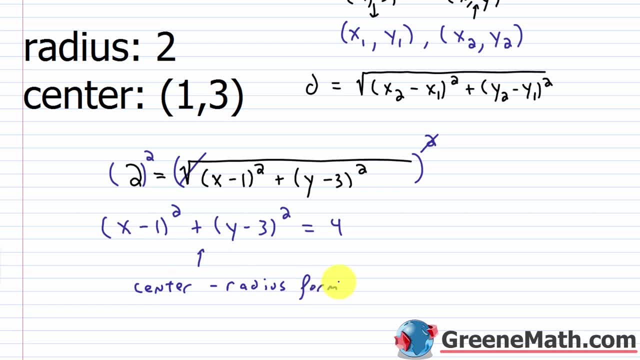 Form- And you might hear this called standard form for a circle. Those two can go back and forth interchangeably, But the key thing here is to understand that your center will be given by this guy and this guy. So as long as it's in the format of x minus something, 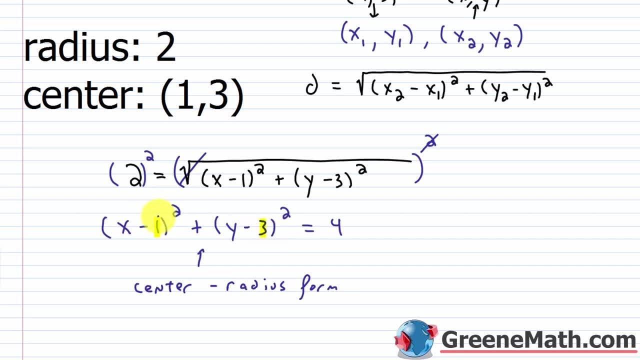 and y, minus something you just take. whatever the number is here and here, and that's how you're going to find your center. So your center here is 1, 3.. We already knew that, because we were given that information. 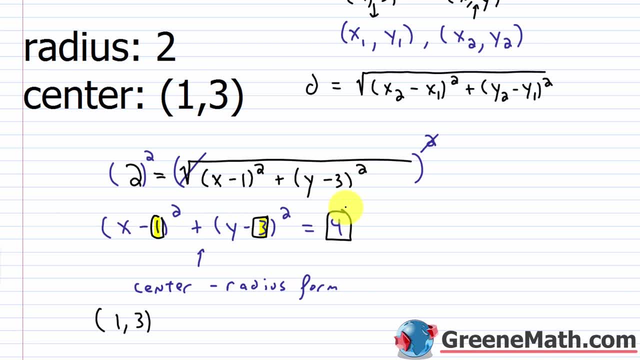 And the radius comes by taking this guy and taking the principal square root of it. So in other words, this right here represents the radius squared. So taking the principal square root gets me back to the radius. Take the square root of 4, I get back to 2.. Now 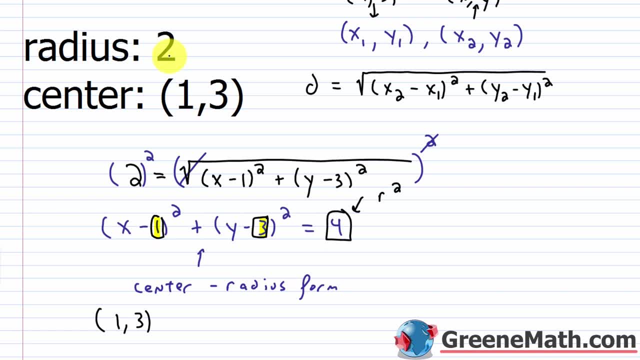 some people will get a little confused and say: well, why don't you take the positive and the negative? The reason we don't say that the radius is also negative 2 is because the fact that a distance has to be non-negative. right, You can't say that, hey, I'm going. 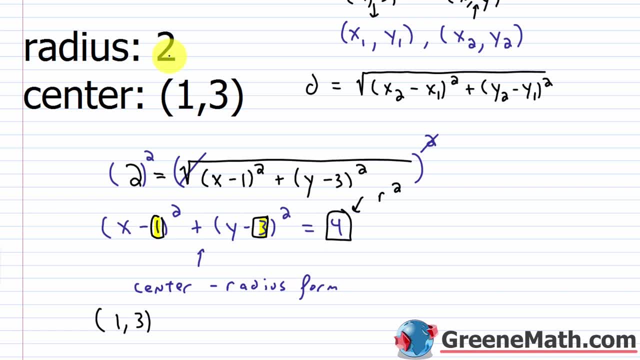 to get in my car and drive negative 2 miles to work. You're either going to go zero miles and not go anywhere, say at your house, Or you're going to go some positive amount right, But you can't just go a negative amount of miles somewhere. 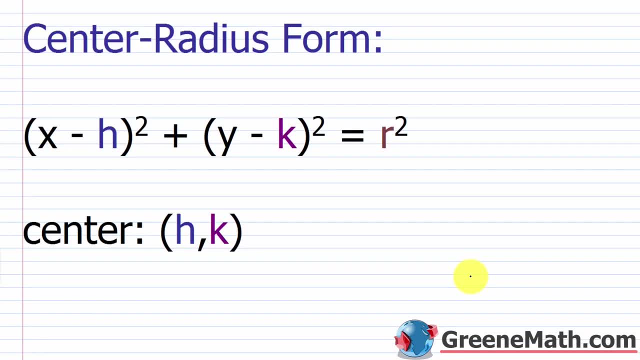 All right. So here is the official formula which you'll see in your textbook. So the center radius form you have x minus some value h squared, plus y minus some value k squared, And this equals the radius squared. So the center is h, comma k and the radius 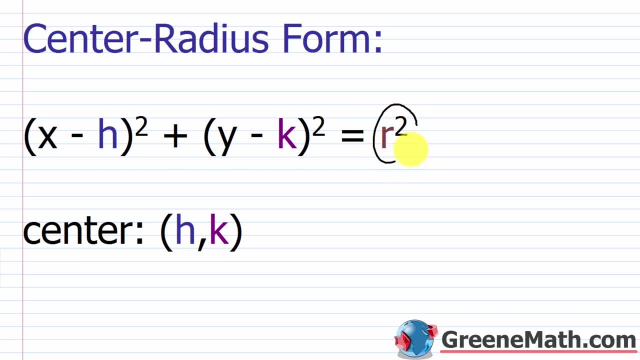 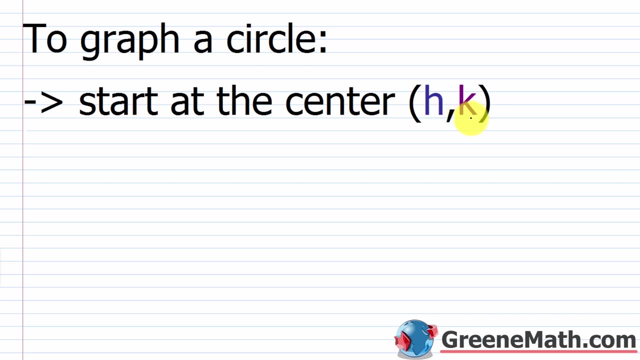 we find again by taking the principal square root of what we see here. So if I know my center and my radius, I can very quickly graph something. So to graph a circle, I start at the center, which is h comma k, I make a nice little clean point, Then I move by. 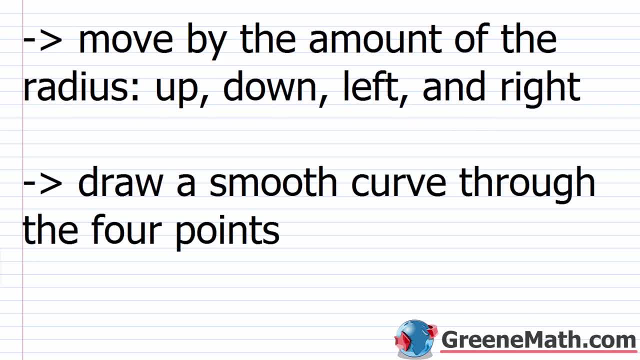 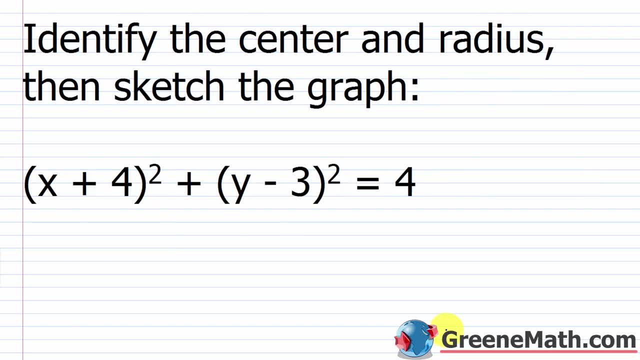 the amount of the radius. So up down, left and right. So you end up just making four nice clean points And then you draw a smooth curve through the four points. So let's look at a few examples. These are things you would see in your textbook pretty much right away. 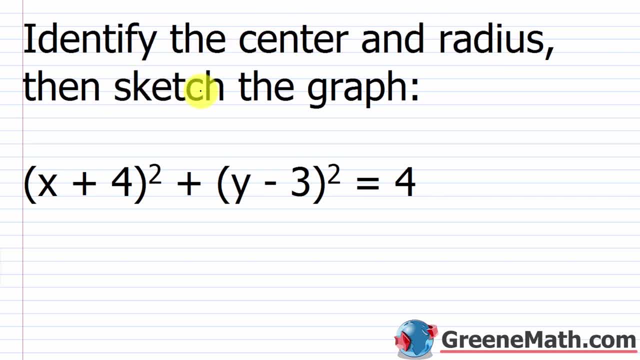 So we want to identify the center and radius. then sketch the graph. So we have x plus 4, that quantity squared plus. we have y minus 3, that quantity squared, and this equals 4.. So again to match the format, we add x minus h, this quantity squared, then plus. 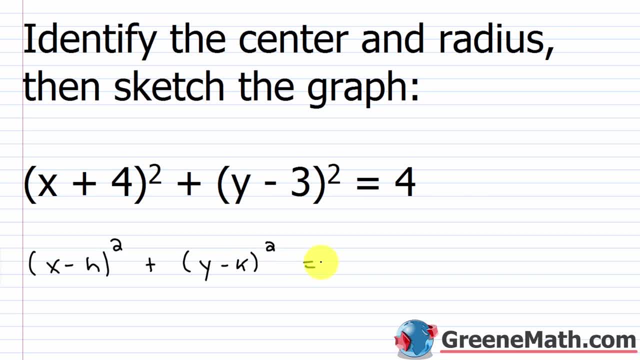 y minus k, this quantity squared, This equals the radius squared. Now here's where you got to pay close attention. This is a minus sign here and a minus sign here. If it's not presented in that exact format. you have to make an adjustment to what you're looking. 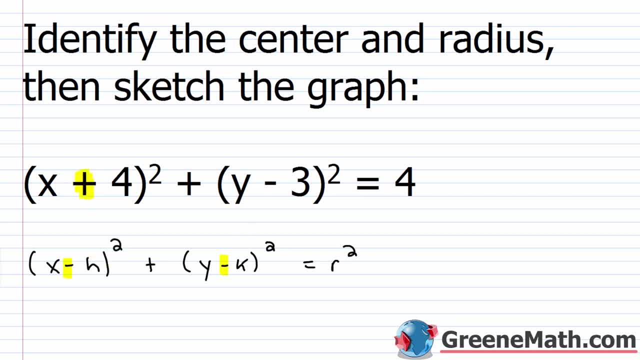 at: This is a plus here. So what I would do is I would say: okay, I can write that as x minus a negative 4.. So in other words, I can say: this is x minus a negative 4.. Now 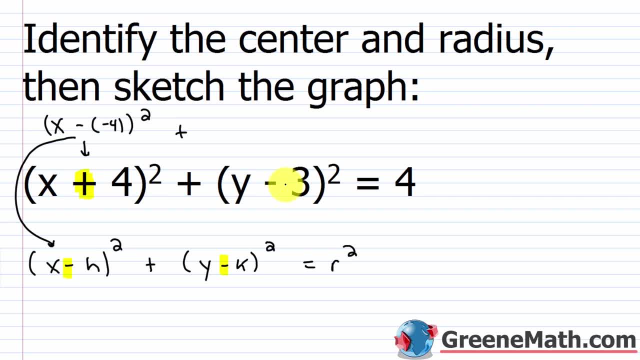 I'm going to write this as 2 squared just to match everything. So now I can just quickly look at the equation and pull the information out that I want. If I want the center again, I match things up: h here, h here, k here, h here. So I'm going to write this as 2 squared. 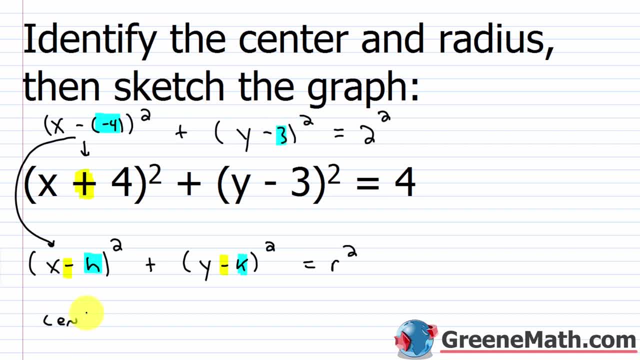 k here. So the center occurs at the point negative 4,, that's my x value, and then positive 3, that's my y value, Then the radius. the radius again. when I take the principal square to 4, I get 2.. That's why I wrote it as 2 squared, So my radius is 2.. Now I can quickly. 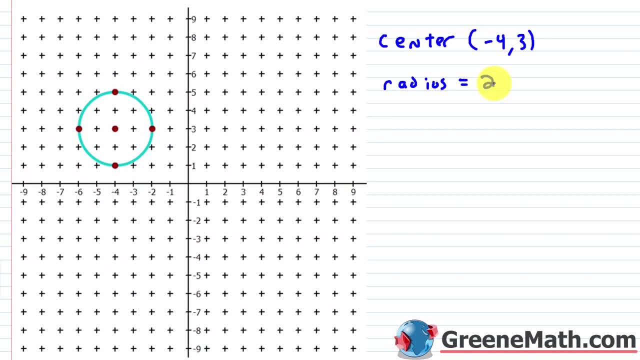 graph this guy with this information. So I've already pre-drawn the circle. as you can see The reason I did that. it's kind of hard to freehand draw a circle, So I'm going to just take my circle. especially if you're using a computer, A lot of people 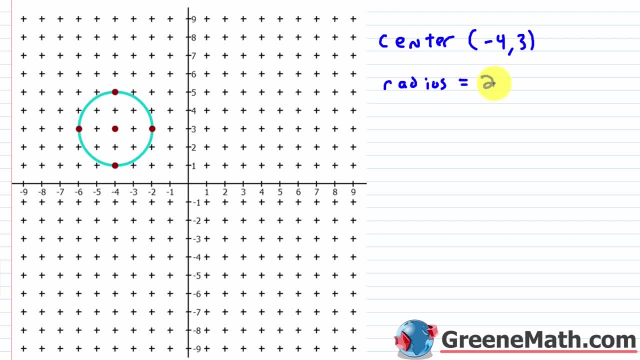 will graph this on their calculator. or if you freehand draw this on a piece of paper, you can kind of stick your wrist down and kind of rotate the page around and make a perfect circle. But if you really freehand draw it it's kind of difficult to do. But 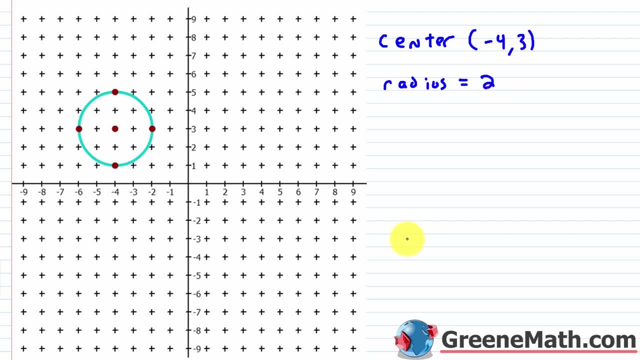 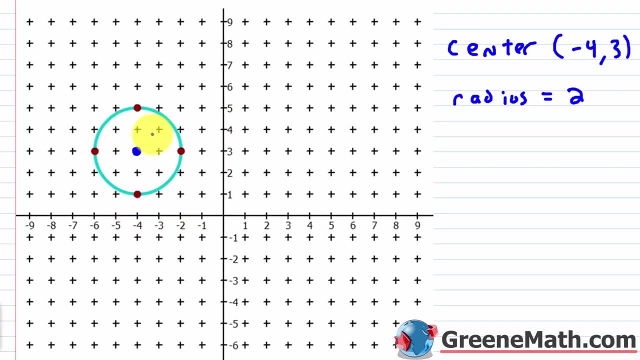 again if you wanted to do this. we're just going to do the exercise. The center is at negative 4,3.. So on the coordinate plane I would go 4 units to the left and 3 units up. So that's why I have that point right there. That's your center. 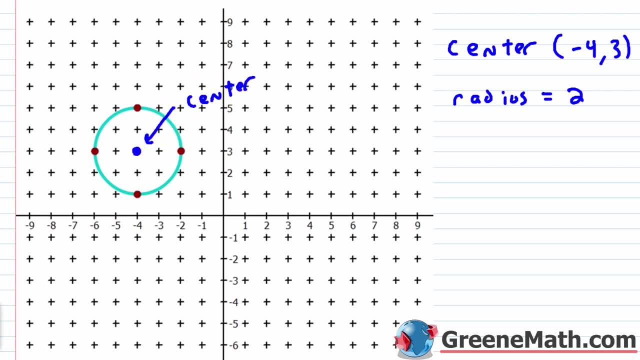 So this is the center and I can just highlight that. And then after that I'm going to make four points. I'm going to go up by the radius, I'm going to go up by two units. So that's right here. 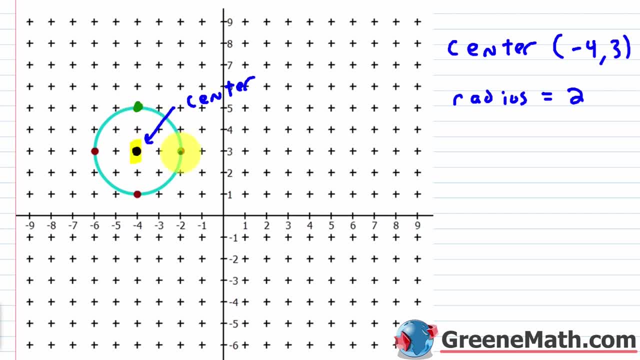 That's why there's a point there: I'm going to go to the right by two units, I'm going to go down by two units and I'm going to go to the left by two units. So that's where those four points came from. 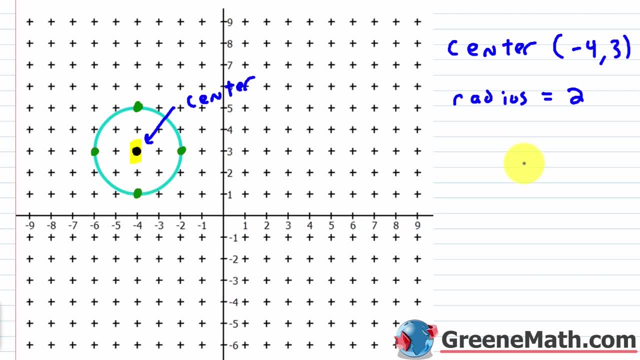 Now, once I've done that, I can just sketch the graph of the circle. I'm going to try to do this to the best of my ability, And that's about as good as I can personally do. I know a lot of people are really good at drawing circles freehand, but personally, 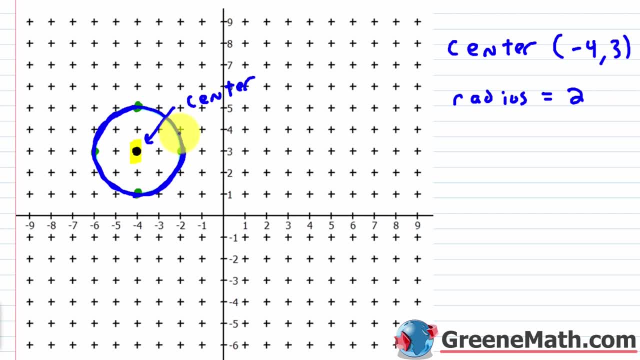 I am not good at it, So that's why I made a graph to kind of start off with. But it's just that easy: Just identify the center. Usually I just make a point And then just move up down to the left and to the right by the radius. 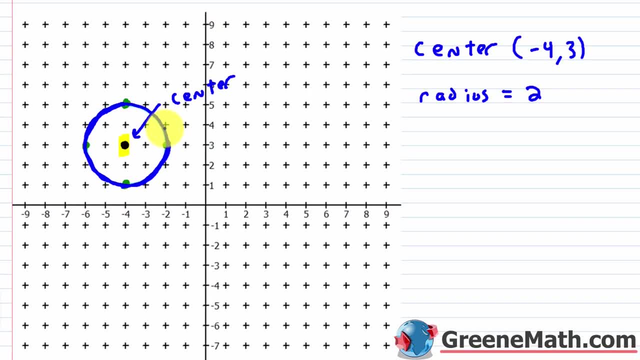 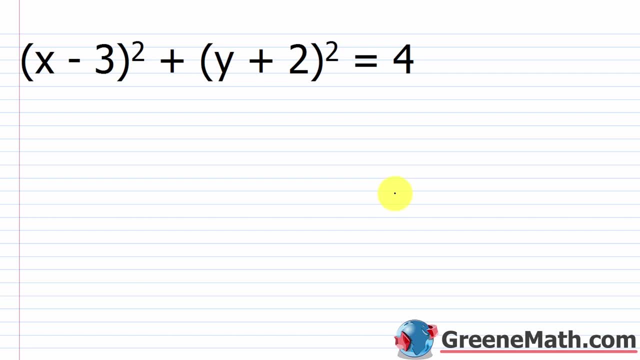 Plot those points and then draw a smooth curve to connect those four points. All right, Let's take a look at this. Let's take a look at another problem. So we have the quantity x minus 3 squared plus the quantity y plus 2 squared. 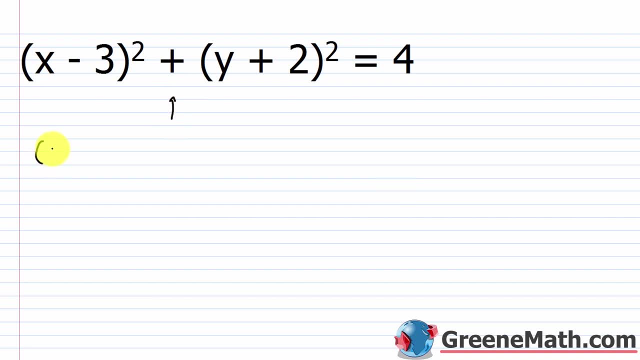 And this equals 4.. Again, match this up to: we have x minus h, that quantity squared, plus we have y minus k- that quantity squared. This equals the radius squared. So I can see that this is minus and this is minus. 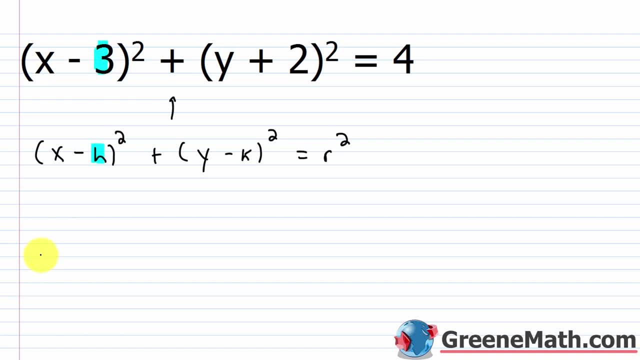 So my h here will be 3.. So if I'm thinking about the center, the x squared, the y coordinate will be 3.. Now for the y coordinate. I have a plus here, So I've got to think about rewriting that. 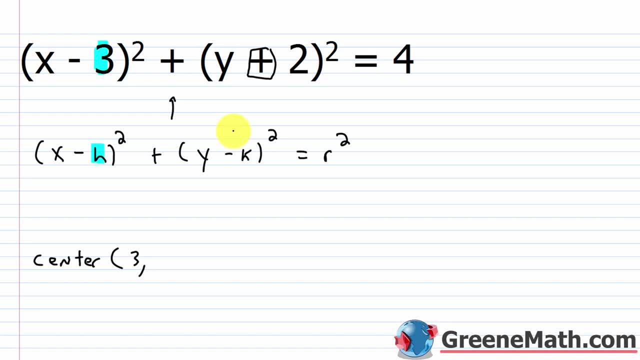 So if it's a plus, this is going to be minus a negative 2 to get it to match that format. So in other words, I can say: this is y minus a negative 2, this quantity squared, Then we can see that k would be negative 2 here. 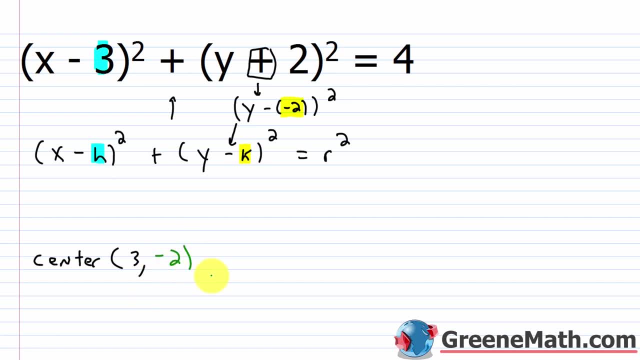 So my y coordinate would be negative 2.. And then what about the radius? Again, you just take this guy here and you take the principal square root. So I can really think about this: instead of being 4, you can say this is 2 squared, right. 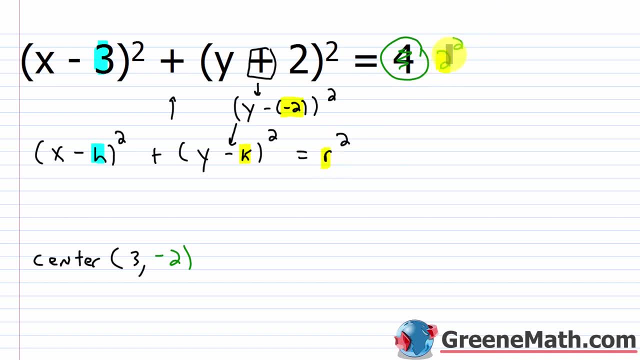 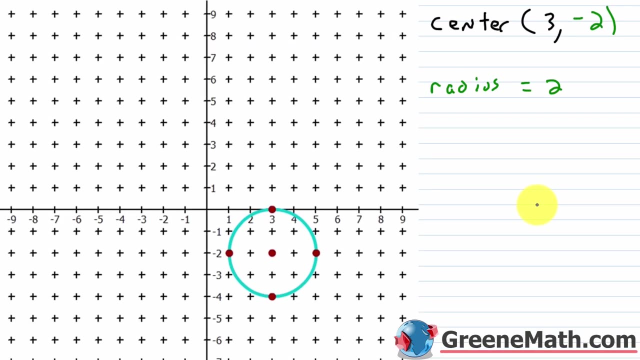 So the radius is just 2.. It's just this part right here, the base of the exponential expression you set up. So my radius is 2.. All right, let's take this information and graph it. So again, the center occurs at 3 comma negative 2, and the radius is 2.. 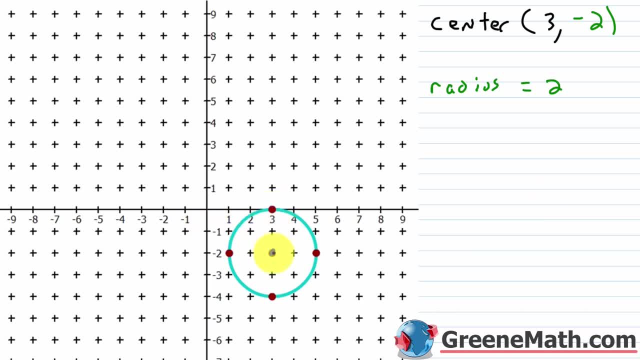 So I go 3 units to the right and 2 units down. This is my center. So again, this is the center. And then I would make 4 points. So I'd use my radius, which is 2, to go up by 2 units, to go to the right by 2 units. 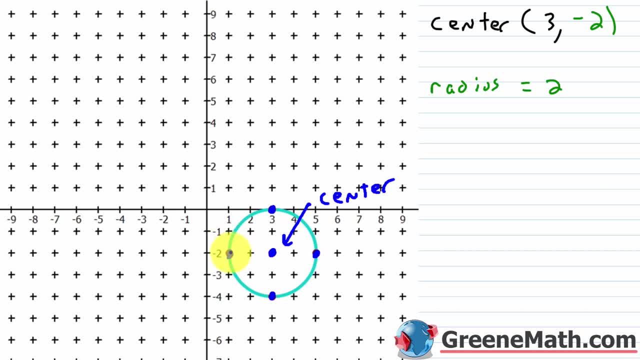 to go down by 2 units and go to the left by 2 units. Once I have those 4 points again, I can draw a smooth curve, or I can attempt to. Not always going to be perfectly smooth, but let's try. 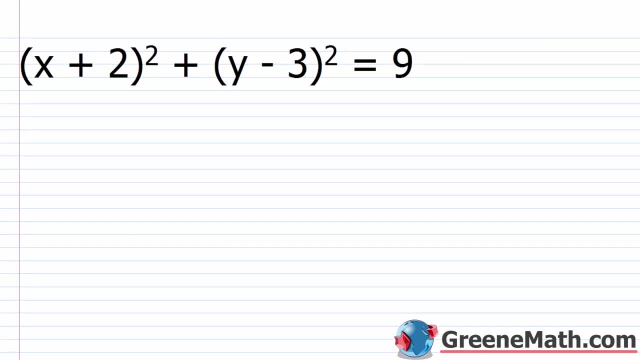 All right, Again, That's about as good as I can personally do. All right, Let's take a look at one more of these easy ones, and then I'll show you a harder scenario, where the information is not given to you in this format and so you have to do a little. 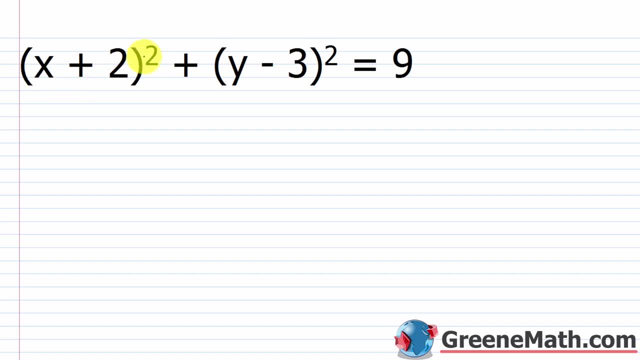 bit of extra work. So here we have x plus 2, that quantity squared. Then plus, we have the quantity y minus 3 squared, and this equals 9.. So again, the format that we're looking at is x minus h, this quantity squared plus. 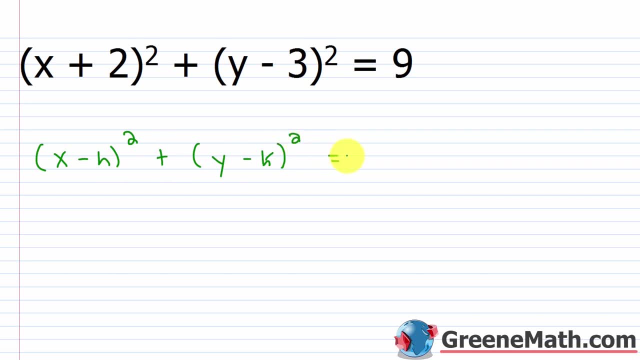 we have y minus k. this quantity squared, This equals our radius. This is squared. So what matches up and what doesn't? This is minus k, this is minus 3.. So 3 here is k, The h here is not 2, because again I have this plus sign here. 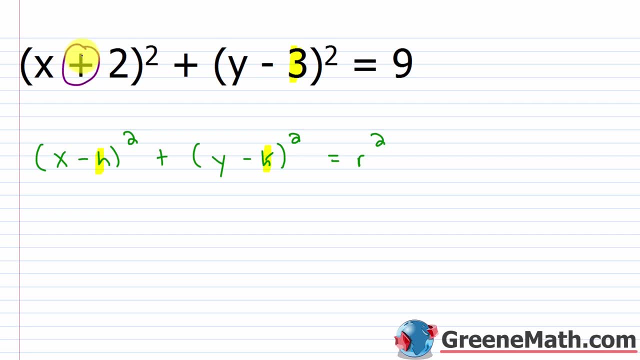 So I've got to account for the formula. If I see a plus sign I can just cross that out and put minus a negative. So I know h is represented by negative 2.. So for the center, for the center we can say this occurs at the point negative 2,. 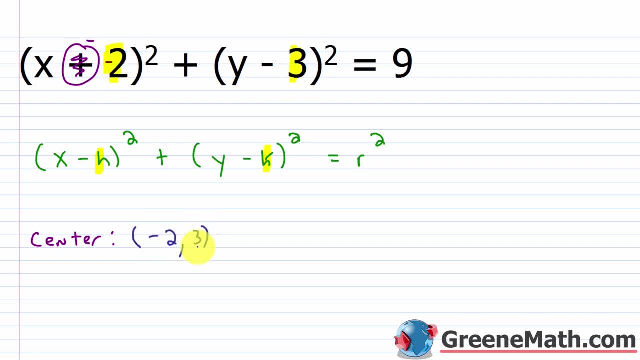 comma 3.. Now for the radius. again, I could take 9, I could just write it as 3 squared, or I could take the principal square root of it and come up with 3, however you want to do that. 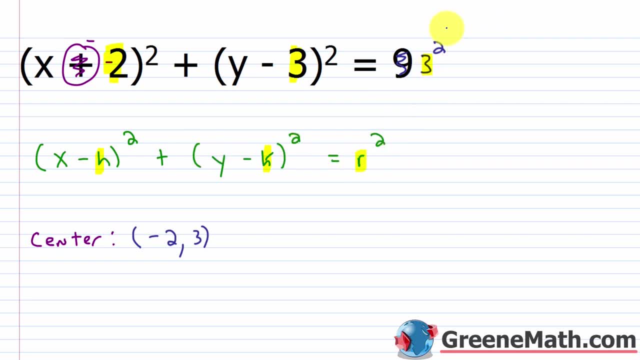 But a lot of people like to just match the formula up exactly. So again, if you set this up as an exponential expression, 3 squared, you know the radius is the base 3.. So I'll put my: radius here is equal to 3.. 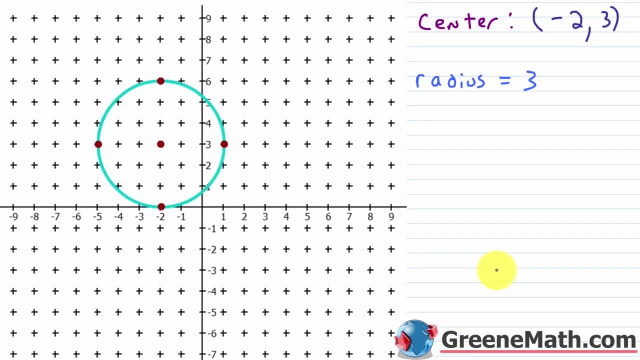 So let's copy this. All right, Our center occurs at negative 2, comma 3.. So I go 2 units to the left and 3 units up. So this is our center. This is our center, And then the radius is 3.. 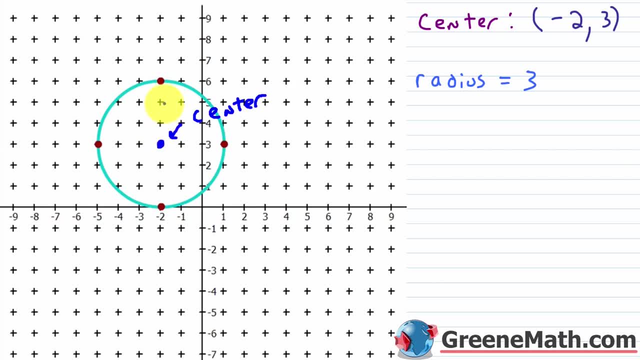 So again, to make those 4 points from the center, I'd go up by 1,, 2, 3.. I would go down by 1,, 2, 3.. I would go to the left by 1,, 2, 3.. 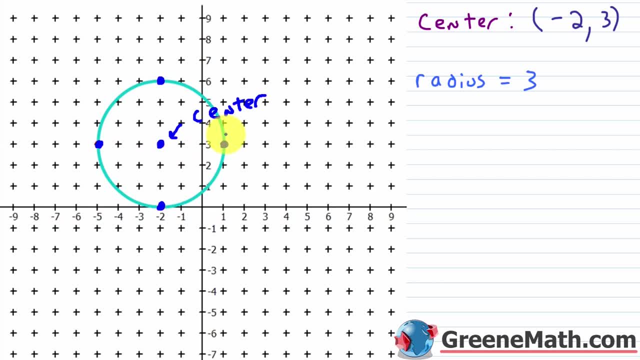 And I would go to the right by 1,, 2,, 3.. So very easy, once I have that, Let me just change colors here and I will again attempt to draw the circle. I'm just going to connect those 4 outer points with a smooth curve. 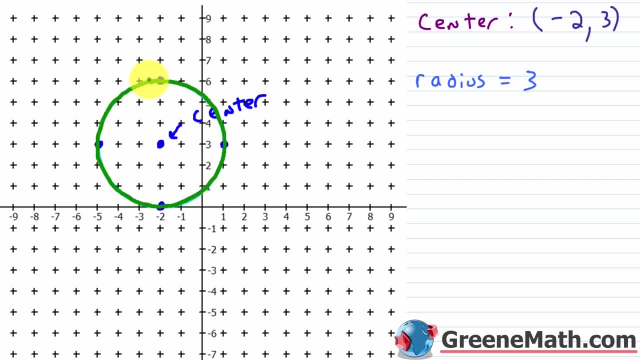 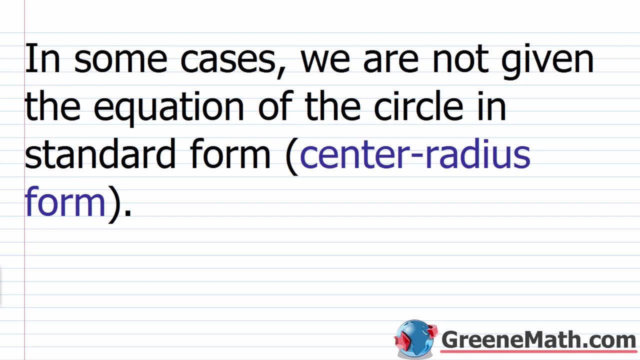 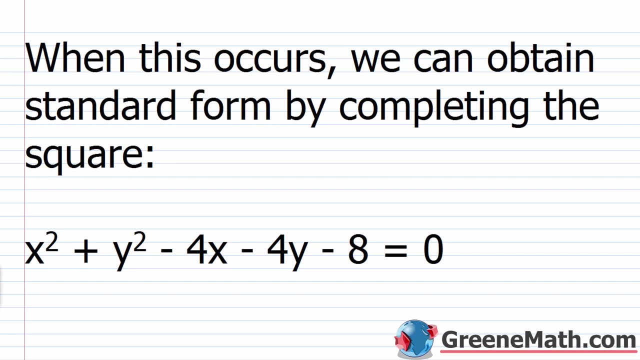 All right. So there is our circle, All right. So in some cases we are not given the equation of the circle in standard form, again otherwise known as center radius form. So when this occurs, we can obtain standard form by completing the square. 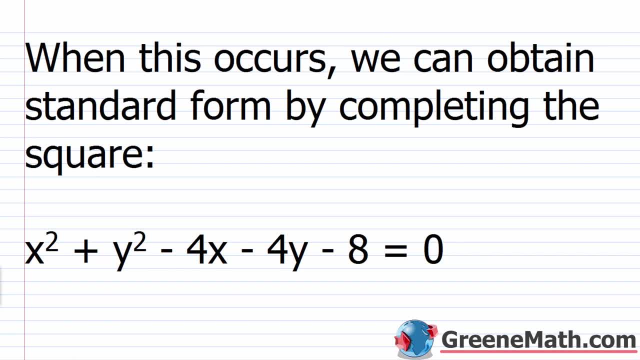 So this is actually quite an easy process. If you remember solving quadratic equations by completing the square, It's kind of the same thing, but it's a lot easier. So essentially all I'm going to do here. if I look at this first equation, we have 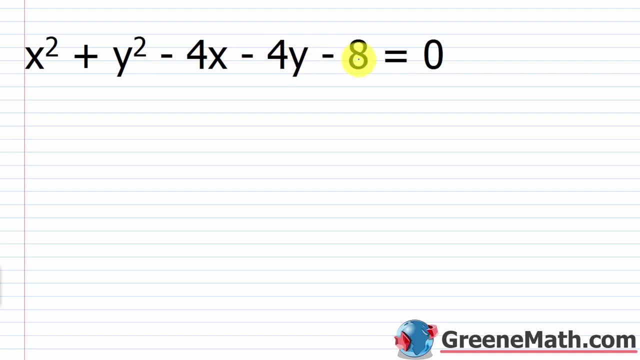 x squared plus y squared minus 4x minus 4y minus 8 equals 0.. The first thing I would do is group my x terms together and my y terms together And I would take the constant and send it to the other side. 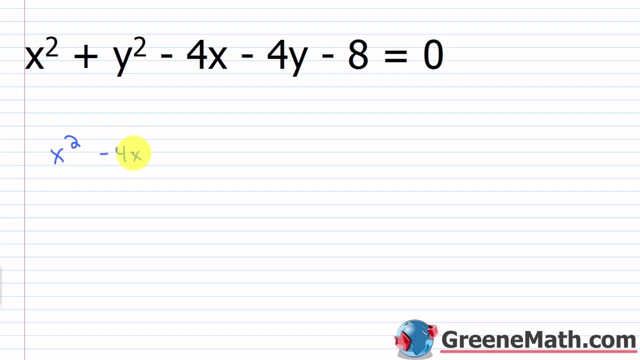 So in other words, I would say this is x squared minus 4x. I would group those two together And then plus I would take the y terms, So y squared minus 4y. Group those two together And then I would add 8 to both sides of the equation. 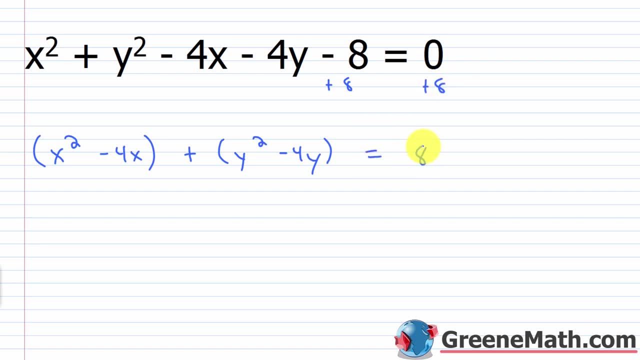 So this equals 8.. Now, if you remember from again that lesson where we completed the square to solve quadratic equations, the steps would be to look at the coefficient on the first degree term, So in other words the variable that is raised to the first power. 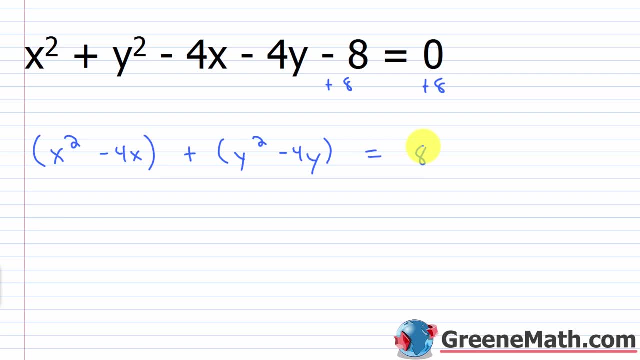 You take that coefficient And you cut it in half, Meaning you multiply it by half And then you square the result. This is what you're going to add to both sides of the equation to complete the square. So very, very easy to do this. 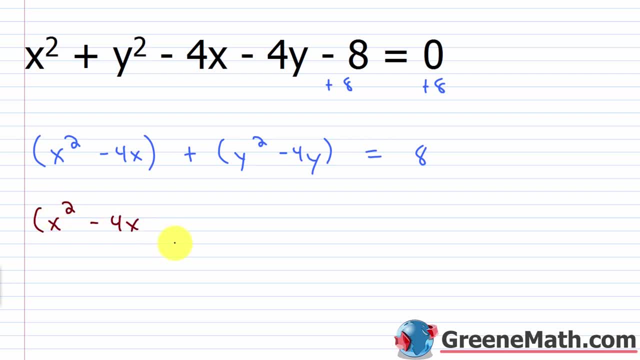 So we have x squared minus 4x To complete the square. here again get a perfect square trinomial, Something I can factor into a binomial squared. I would take this coefficient right here, So it's negative 4.. 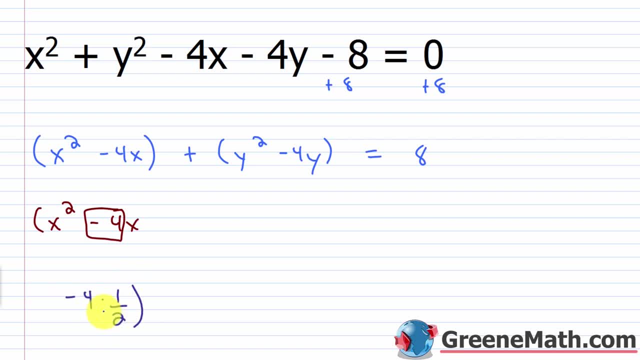 I would cut it in half, So I'd multiply it. I'd multiply it by half And then I would square it. Negative 4 times a half is negative 2. Negative 2 squared is 4. So I would add 4 here. 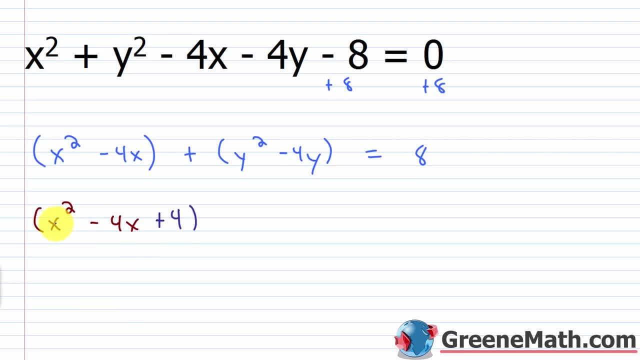 Now this gives me a perfect square trinomial. This would factor into x minus 2, that quantity squared. Here's the issue, though I added 4 to this side of the equation, So I can't just do that. I have to balance it by adding 4 to this side of the equation. 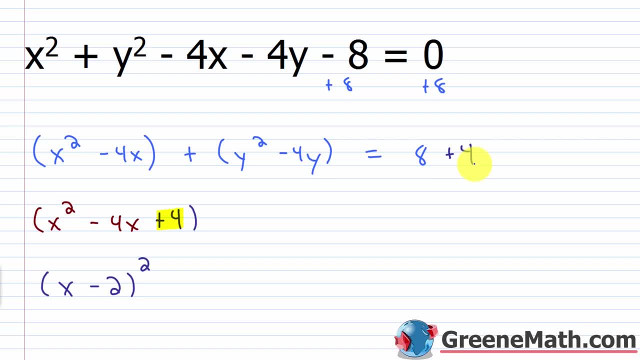 So I can't just do that, I have to add 4 to this side of the equation as well. As long as I do that, everything is okay. So then, plus, We're going to do the same thing over here. So we have y squared minus 4y. 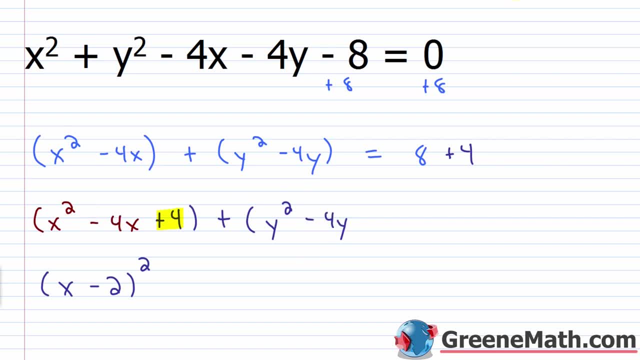 Now this coefficient here is the same as the coefficient here. I had a negative 4 here and I have a negative 4 here. So without even doing the work of saying negative, 4 times a half that amount squared, which gives me 4, I can just look here and know that I would add 4 to this side over here. 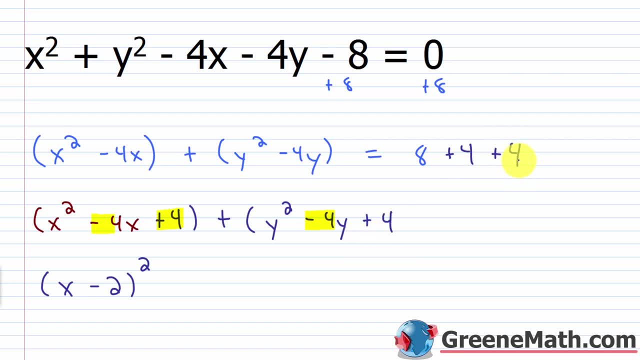 And again doing that, I have to also add 4 over here, just to make sure it's balanced. So this is plus. We know this would factor into y minus 2, that quantity squared Over here, 8 plus 4 is 12, 12 plus 4 is 16, so this equals 16.. 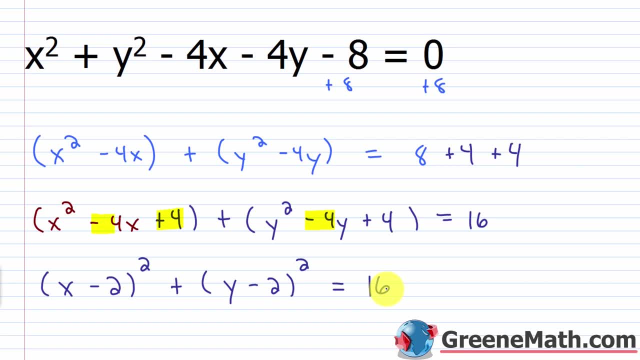 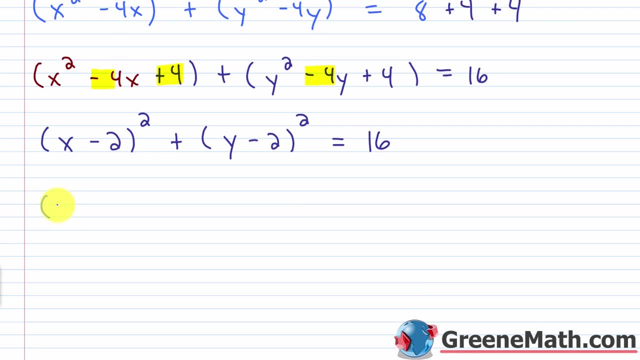 Now you have this in center radius form or standard form, however you want to think about it, So we can look at again. I can match this up with x minus h, that quantity squared. So we have x minus h, that quantity squared. And again doing that, I have to also add 4 over here, just to make sure it's balanced. So that's why this many equals small tässä. Then I can't substitute both of those, and the solved equation would be theitta squared. 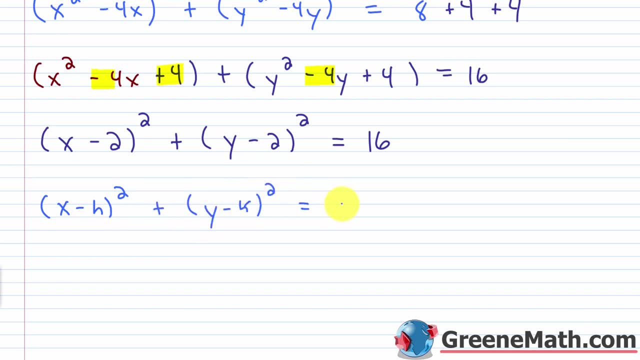 plus y minus k, that quantity squared equals the radius squared, So in this case it's basically perfect. The only thing I would do is I would write 16 as 4 squared, to match up the h with 2, the k with 2, and the r with 4.. 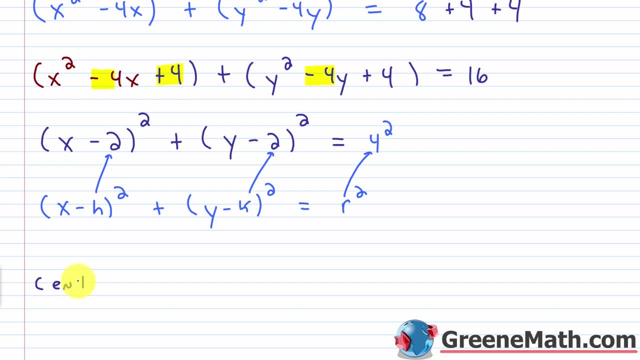 So my center, my center, would occur at the point 2 comma 2.. And my radius, my radius, 2 comma 2.. radius would be four. Okay, very, very simple, Let's take this down to the coordinate plane and 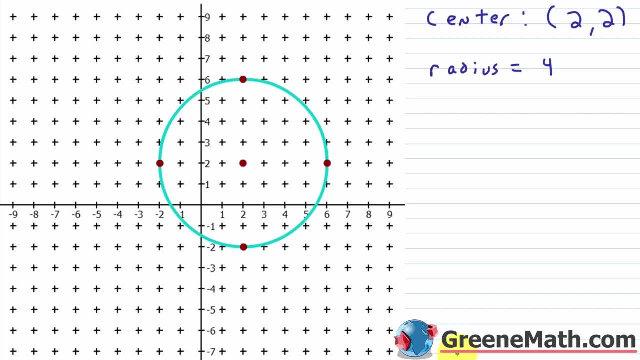 we'll graph this guy real quick, All right, so again, the center here is at two comma two. So two units to the right and two units up. That puts me right there Again. this is my center And then the points we would generate here. the radius is four, So I could go up one, two, three. 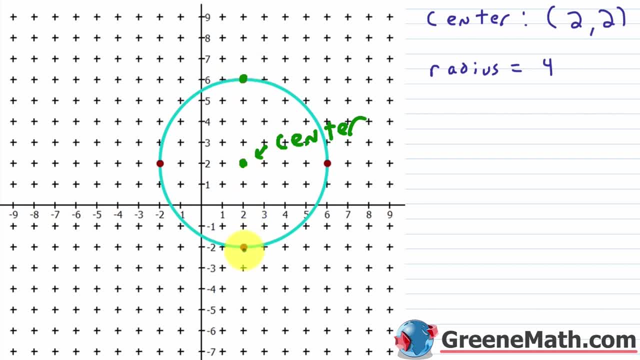 four. There's a point. Down: one, two, three, four. There's a point. To the right: one, two, three, four. There's a point. And then to the left: one, two, three, four. There's a point. 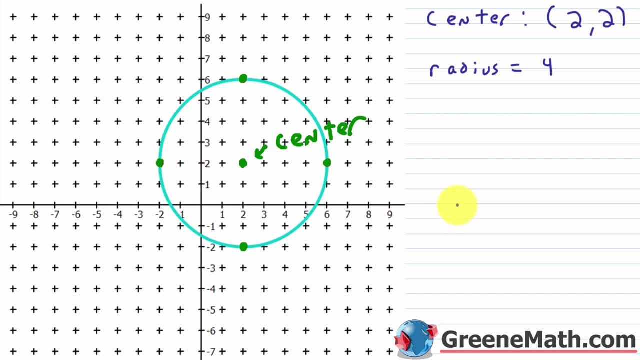 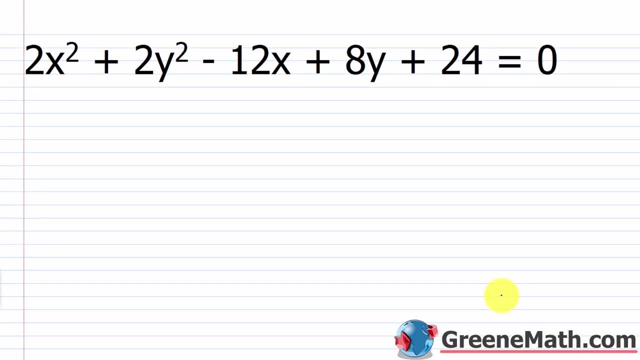 Again, I just want to draw a smooth curve through the points. I'm just going to try to trace this guy that I've already pre-drawn. All right, let's take a look at one more problem here. So we have two x squared plus two y squared, minus 12 x plus eight y plus 24 equals zero. 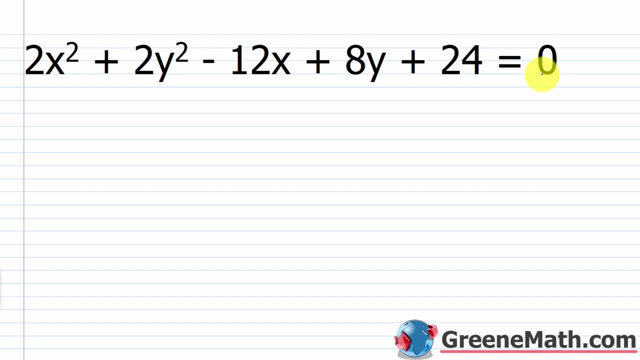 The first thing you would notice before you do anything here is that everything's divisible by two. So if I went through and divided everything by two, what would I get? This would be x squared plus. this would be y squared. Then minus, we'd have six, x plus we'd have four y plus we'd have. 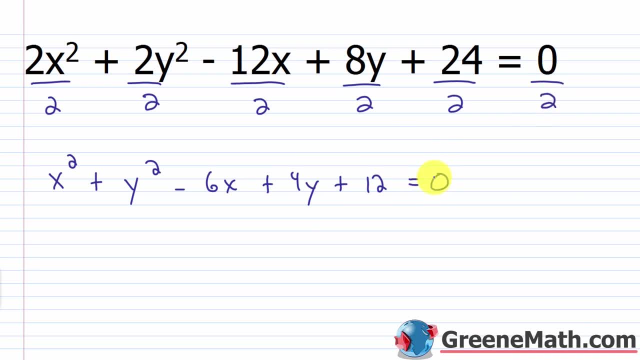 12, and this equals zero over two is zero. Now again, to complete the square. the first thing I'd want to do is I want to grab all my x terms and group those together, all my y terms and group those together, And I want to put the constant on the other side. So I would say this is x squared. 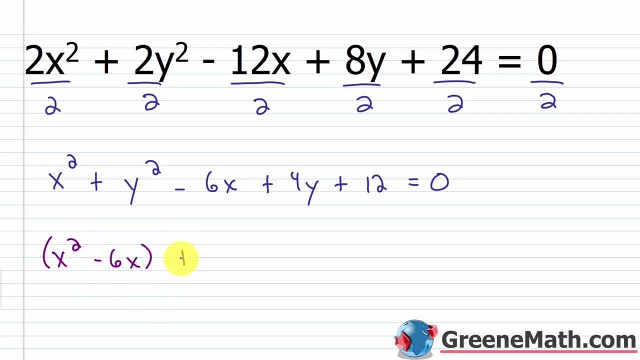 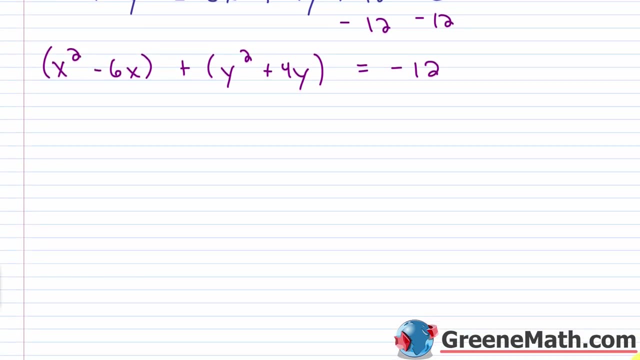 minus six- x- group those together. Then plus, we'd have y squared, plus four y- group those together, And I would subtract 12 away from each side of the equation. So this equals negative 12.. Okay, so now we're going to complete the square. Again, I'm going to choose. 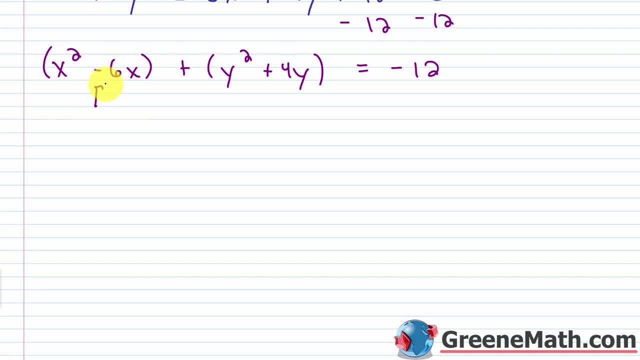 something that takes that binomial there, makes it into a trinomial that can then be factored into a binomial square Again. perfect square trinomial means it's a binomial square if we factored it. All right. so what do I need to do here? So this is x squared minus six x. What's the missing part? 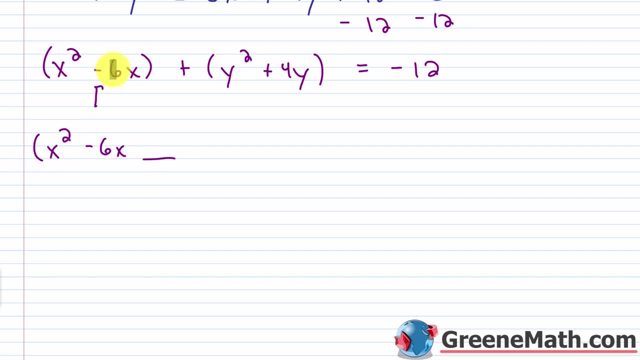 there Again. I take the coefficient for the variable that's raised to the first power. In this case that's going to be negative six. I cut it in half. So I take negative six and I multiply it by a half And then I square the result: Negative six times one. half is going to be negative three. 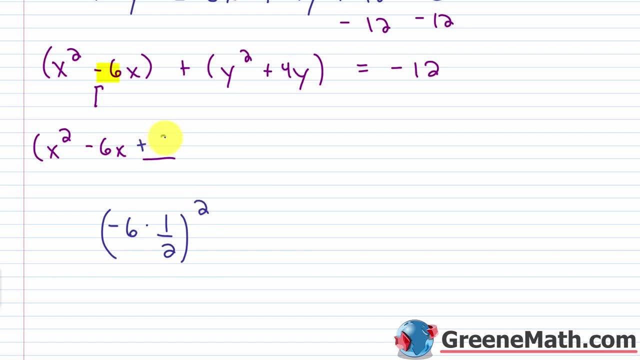 Then negative three squared would be nine. So I'm going to add nine over here. But again, to make this legal I've got to add nine over here. So that part's done. We'll close the parentheses here And then we can go ahead and factor, because we know this would factor. 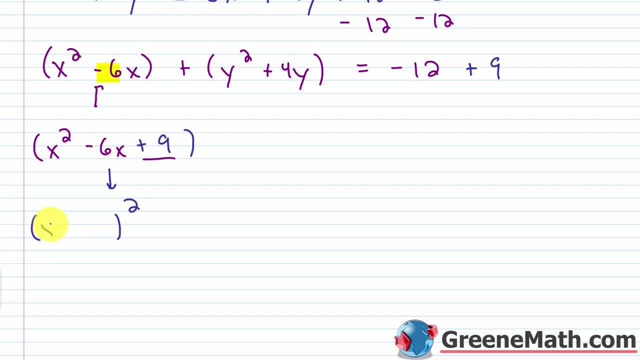 into a binomial square. This would factor into x minus three, that quantity squared, All right. so then plus over, here we have y squared plus four y, And then you have something that's missing here. So again, if I cut four in half, in other words if I multiply four by a half, 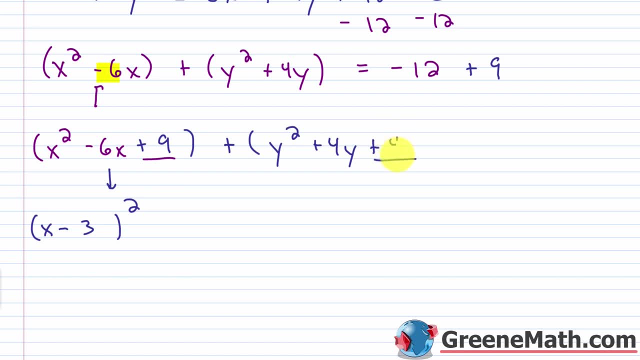 I get two Square two, I get four. So I'm going to add four over here. I'm going to add four over here. So this makes this into a binomial squared which is going to be y plus two, that quantity. 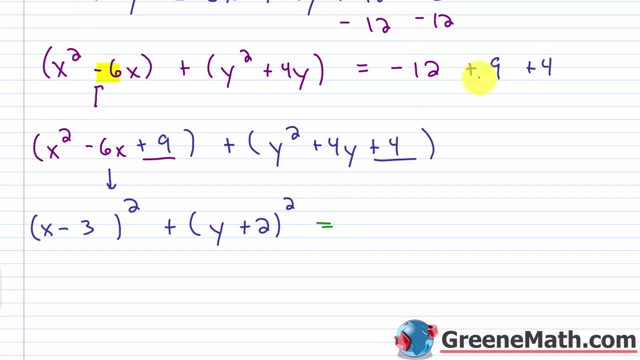 squared. Okay, then this equals negative 12 plus nine. This is going to be negative three. Negative three plus four is one. So to put this into our format, I'm going to write this as x minus three, that quantity squared. This has a minus sign here. 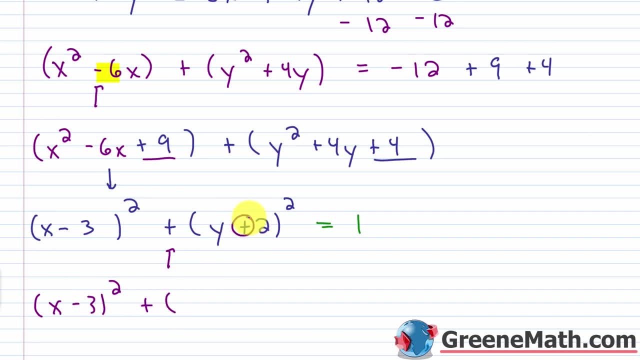 So we're good to go. Then plus over here I'm going to change this to minus a negative, So y minus a negative two. So now we're good to go. there, That's squared. And this equals. you could say: this is one square right, Because one to any power is just going to give you one. So I know the. 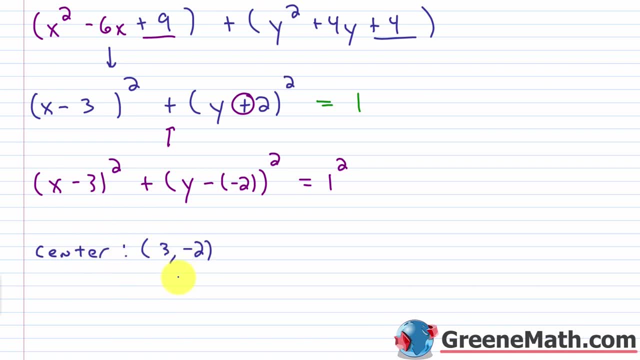 game sounds a little bit calcium, And so you lineed to add some more. Okay, So we're gonna add another two pi times pi times x one, And that's going to make it a negative eight. Okay, And I'm going to write this down. Therefore, I'm going to write down the will be-srix, Okay, So, 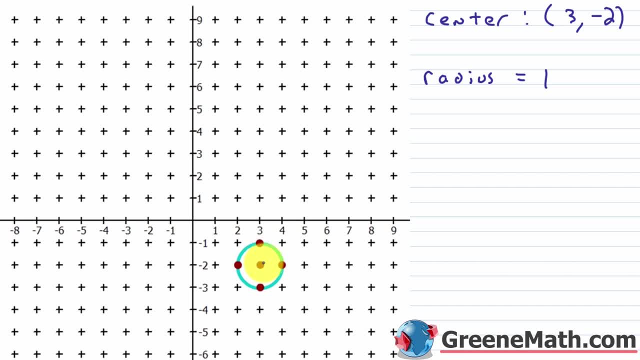 let's look at the defaultせicom negative two. So whatever we're telling myself, if we get three units or less on the center of the surface, there's still a point down there. So say, meters over here, and we're going to write the feeling down here: Yep, raise your index to 2.. And then 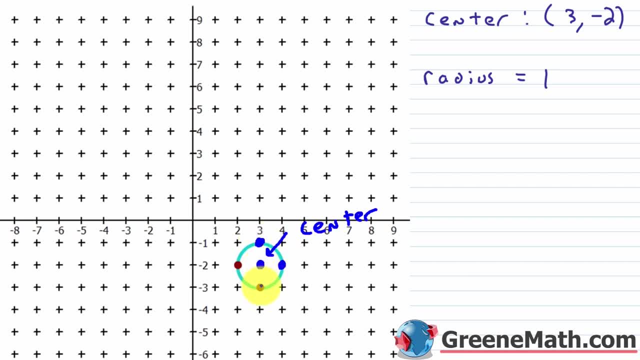 one, I could go to the right one, I could go down one and I can go to the left one, And then I just want to connect the points on the outside with a smooth curve. So don't worry too much about having a perfect graph. 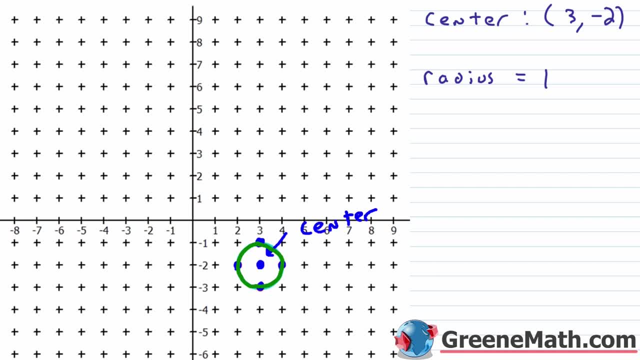 Again, the whole idea here is just to get the concept down, Identify the center, identify the four points on the outside by using the radius and sketch a graph through it and you'll have a good idea of what the circle looks like. 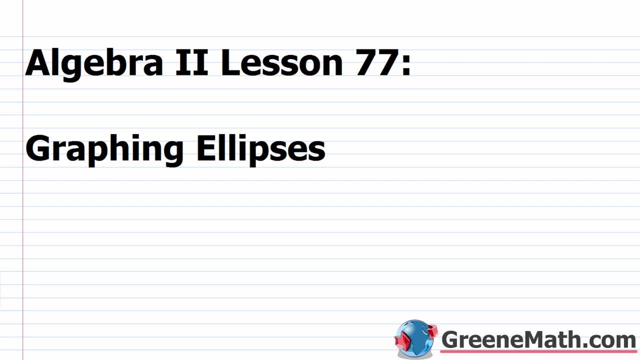 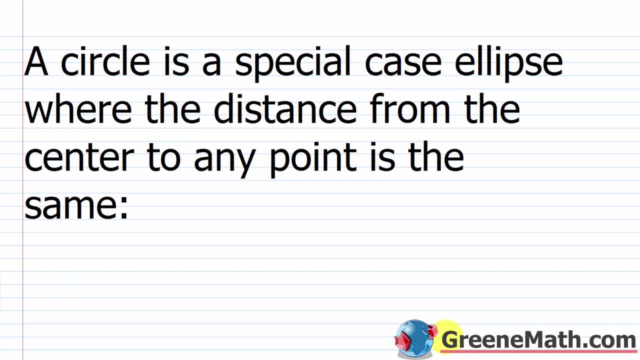 Hello and welcome to Algebra 2, Lesson 77.. In this lesson we're going to learn about graphing ellipses. So in the last lesson we learned how to graph a circle. So it turns out that a circle is just a special case ellipse, where the distance from the center 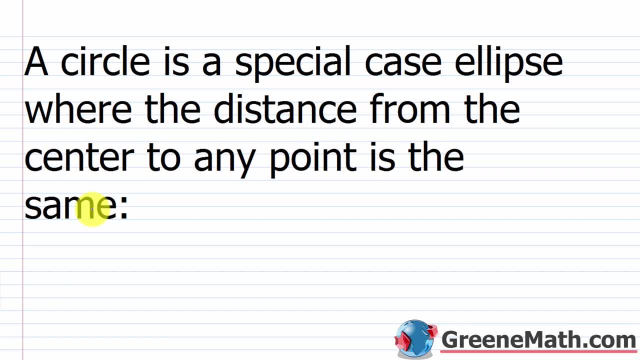 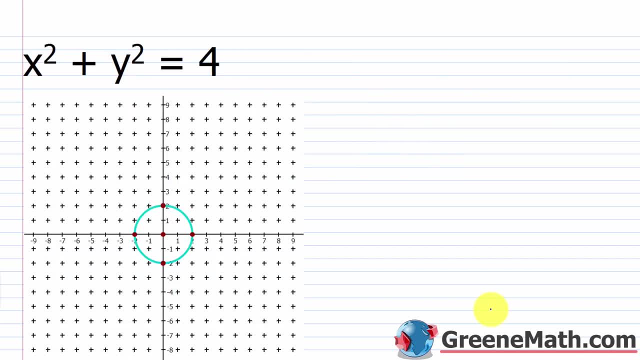 to any point is the same. Now, remember, we had a special name for this distance from the center to any point. We called this the radius. So kind of looking back on that lesson, we saw that if we had a circle that was centered at the origin, it followed. 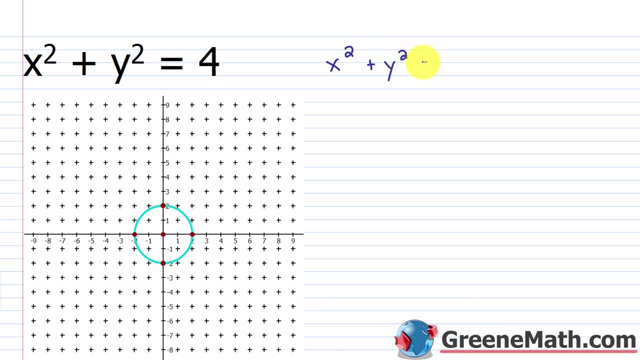 the equation: x squared plus y squared equals r, which stands for the radius squared. So if I looked at x squared plus y squared equals 4, I know this is the radius squared. So if I wanted the actual radius, I would take the principal square root of that and 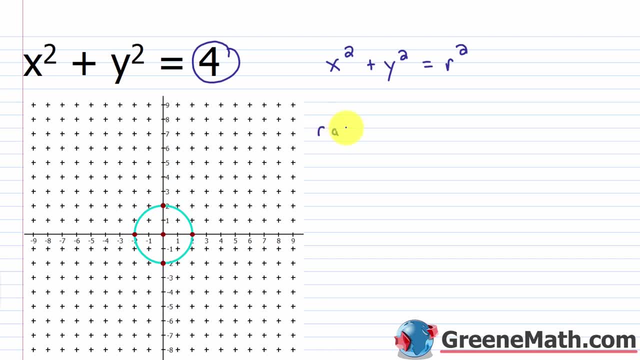 that would give me 2, right Square root of 4 is 2.. So my radius is equal to 2.. Now I already told you, this is centered at the origin, So we can say our center is at 0 comma 0.. 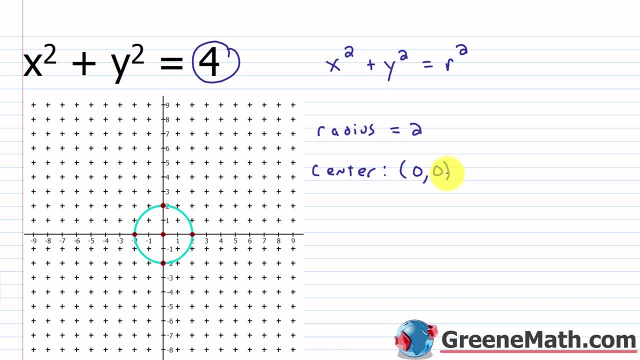 But the way you can tell it's centered at the origin. if you just have x squared and you just have y squared, So you don't have x minus something or x plus something, And that's squared. You don't have y minus something or y plus something squared. 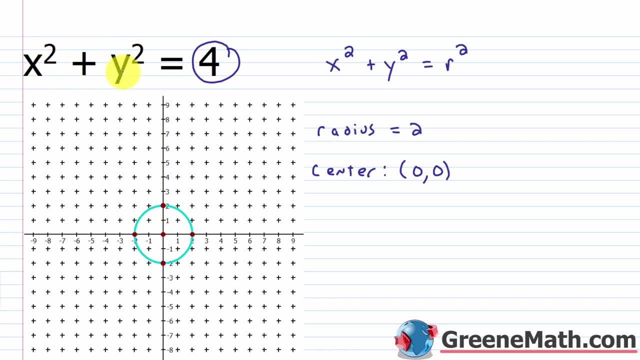 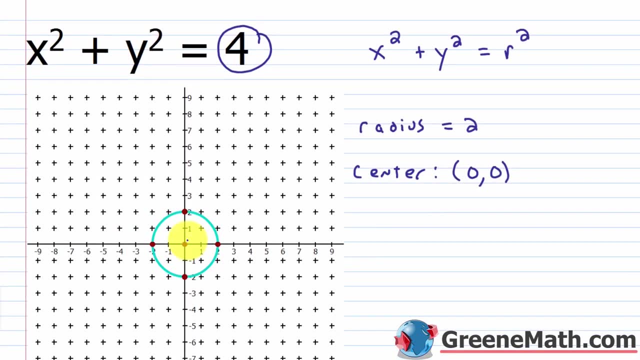 When you just see x squared or y squared, this guy is centered at the origin. So to graph the circle, We lead extra coefficients. Rep Tamera verdad, caber pedira learned that we started at the center. In this case, that's at zero comma zero. so that's right there. 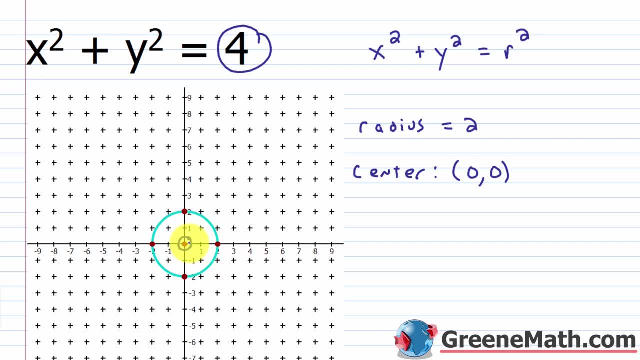 Then remember, the radius is a distance from the center to any given point on that circle. What we can do is start at the center and move to the right by the radius and make a point. We can move up by the radius and make a point. We can move to the left by the radius and make 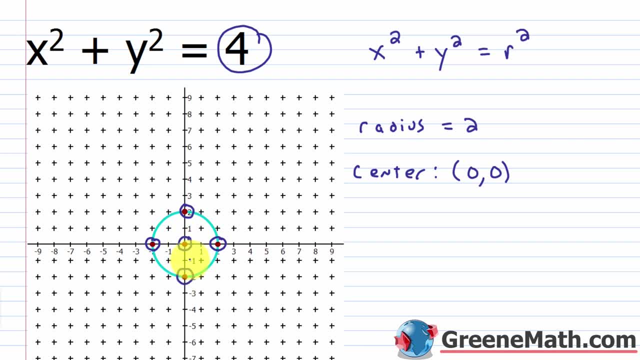 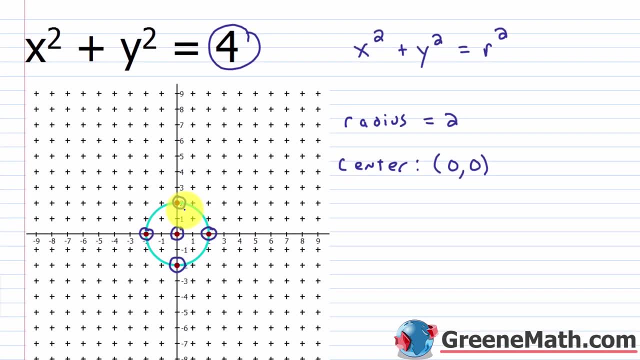 a point And we can move down by the radius and make a point. So once we have those four points there, we can sketch a smooth curve through the points and we've just graphed our circle. Then as we move into circles a little bit more, we see that not every circle is centered at the origin. 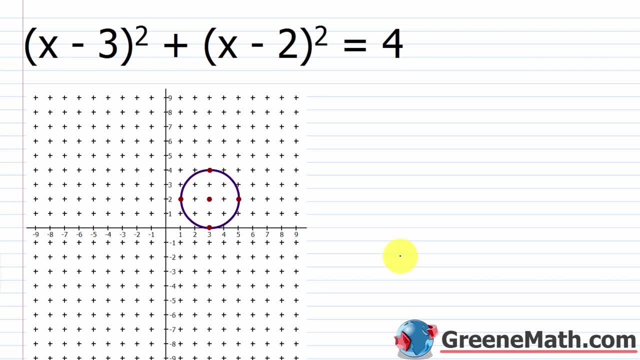 So if we deal with a circle that's been shifted, then what happens is we have the equation x minus h, this quantity squared plus. we have y minus k- that quantity squared. this equals the radius squared. So to think about where the center would have moved to if it follows this format where you have a 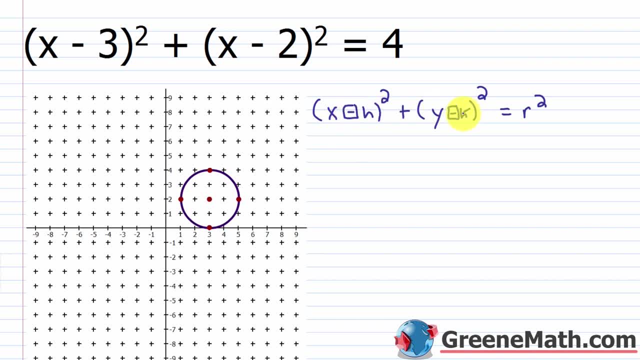 minus some h and then you have a minus some k, the center will occur at h comma k. So in this case, where we have the quantity x minus three squared plus the quantity x minus two squared equals four, where's my center going to be? My center will have moved to three comma two. 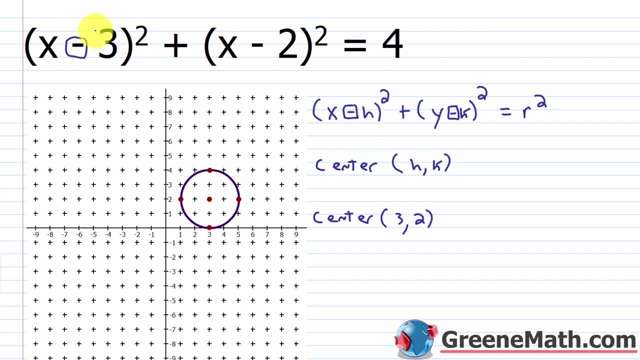 Again, when it matches this format. I have a minus here, So I'm just going to take this three and that's going to be my x value. Here I have the same format. so minus something Here, I'm going to take that two and that's going to be my y value. If you run into the scenario where you have a plus sign, 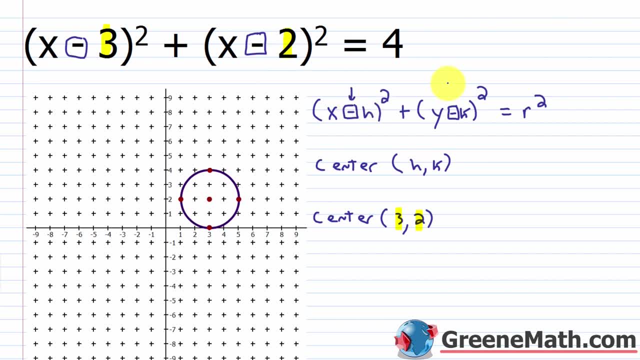 you need to convert it into minus some negative value. That way it matches that formula. Okay, so you have to do that. But this guy, it has the same radius as the last one we looked at. If I take the principal square root of four, I get two, So the radius is equal to two. So essentially, 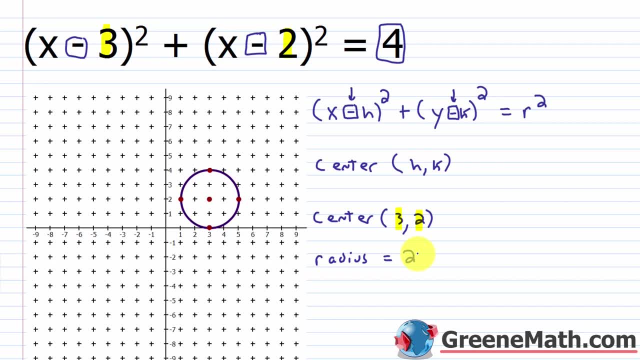 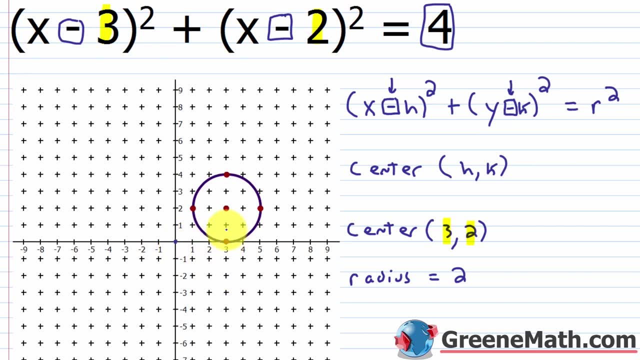 everything is the same. it's just been shifted three units to the right and two units up. My center was right here at the origin, but it moved one, two, three units to the right and one, two units up. So this is my center now And all the other points did the same thing. But again, when you're. 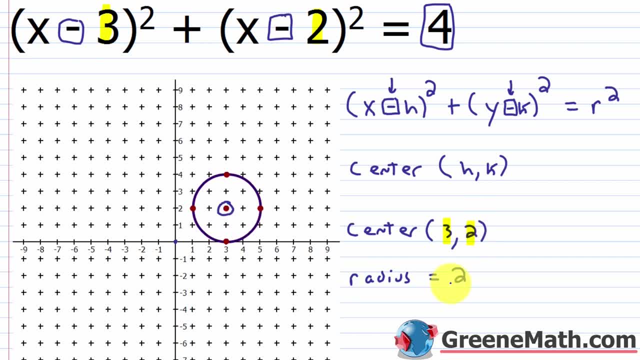 graphing this guy. you just want to look at the center, which is 3 comma 2.. And then again you make your points with your radius. So I go two units to the right, make a point. Two units up, make a point, Two units to the. 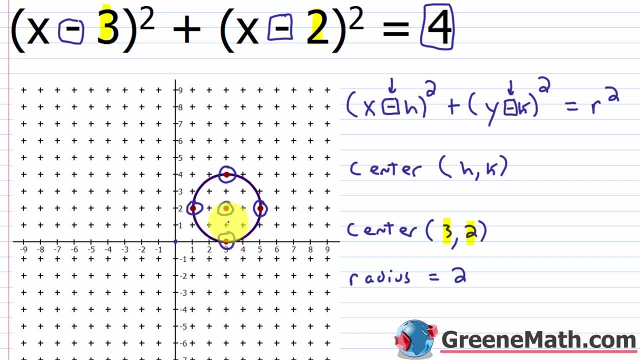 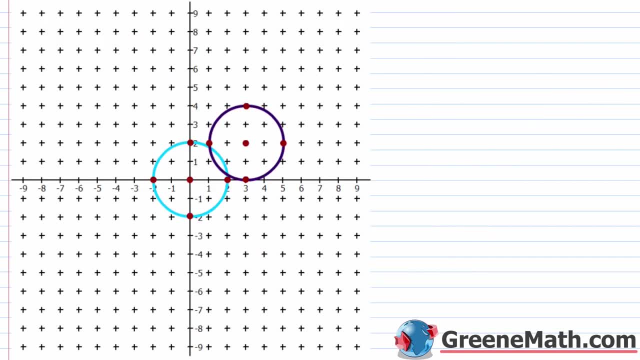 left- make a point. Two units down- make a point. And then I sketch my smooth curve through the points. Now I just want to show you this one so that you can see how it shifted. So, given the fact that they both have the same radius of two, this guy right here again has been shifted three units. 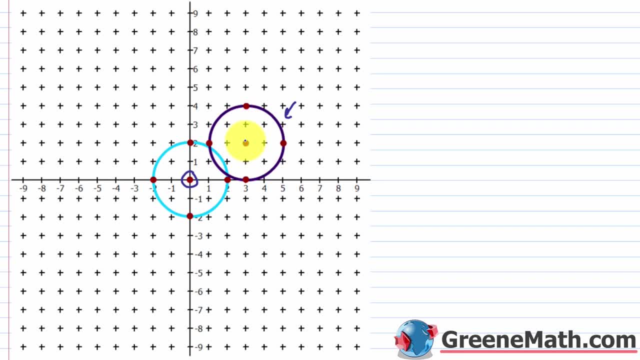 to the right and two units up. So my center went from here to here, Three units right, two units up. You can take any given point. So you can take this point right here and say I went one, two, three units to the right, one, two units up. The impact here again is that for a given point that was on 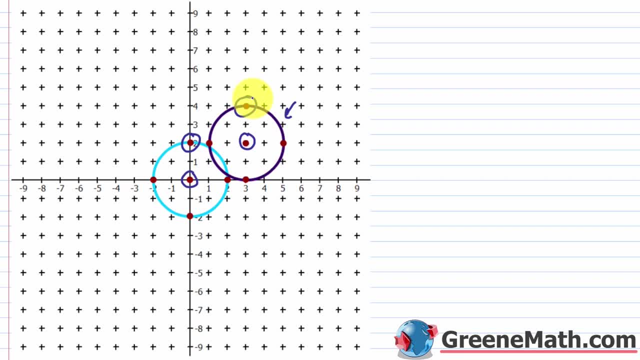 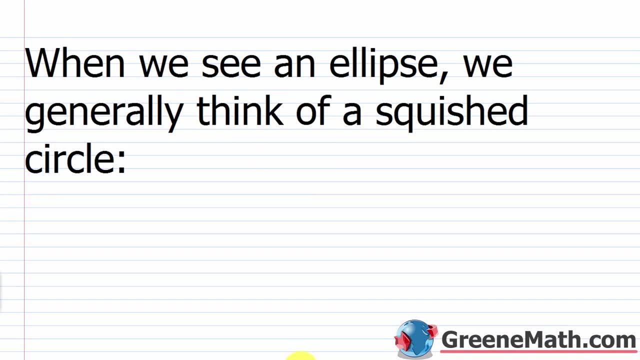 that original graph that we looked at, x squared plus y squared equals four. it's now been moved three units to the right and two units up. All right. so now that we understand the basis of how to graph a circle, we want to move into the ellipse. So graphing an ellipse is not any more difficult. 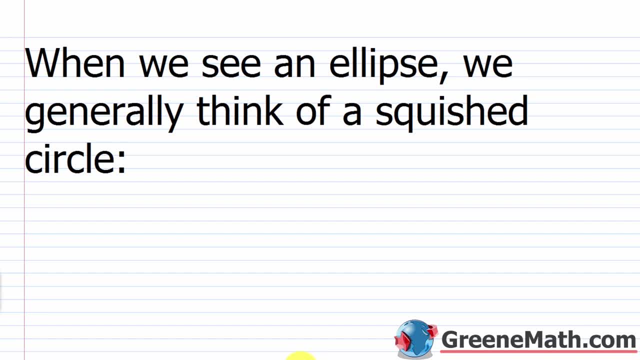 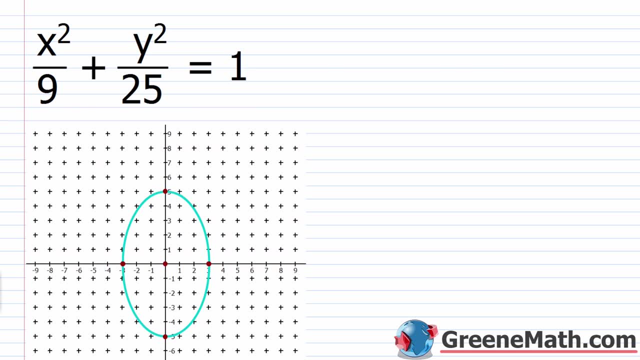 than drawing a circle. Once you learn how to graph a circle, graphing the ellipse is pretty easy. So when we see an ellipse, we generally think of a squished circle. So it may be tall and skinny in the case of a vertical ellipse, or it may be short and fat in the case of a horizontal ellipse. 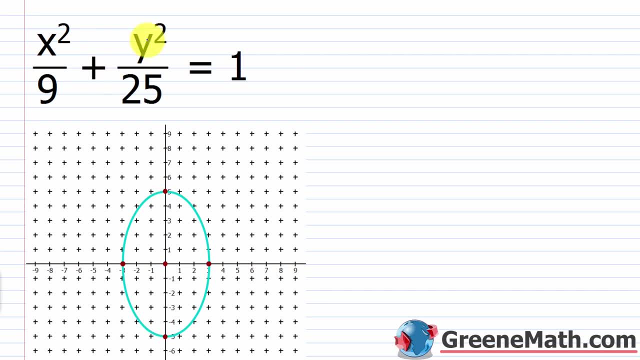 So the first ellipse we're going to look at is x squared over 9 plus y squared over 25 equals 1.. So this type of ellipse is known as a vertical ellipse. You can see that it's tall and skinny And you'll see an example in a minute where it's going to be short and fat, But this guy is a. 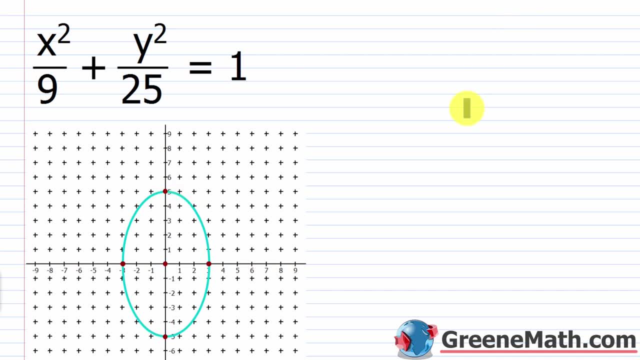 vertical ellipse. I want you to notice something. This is what makes this a vertical ellipse. This guy right here, this 25- the denominator under the y squared is larger than this 9 here, The denominator under the x squared. Think about the fact that y is the vertical axis. 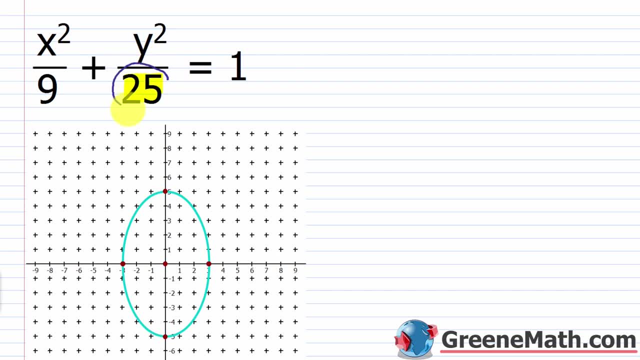 Okay, it's the vertical axis, So when this guy is bigger, you'll get a vertical ellipse. I want you to notice something real quick. Let's say that I told you we wanted to find the y-intercepts here. How would we do that? We'd plug in a 0 for x, So this would go away. I'd have y squared over 25. 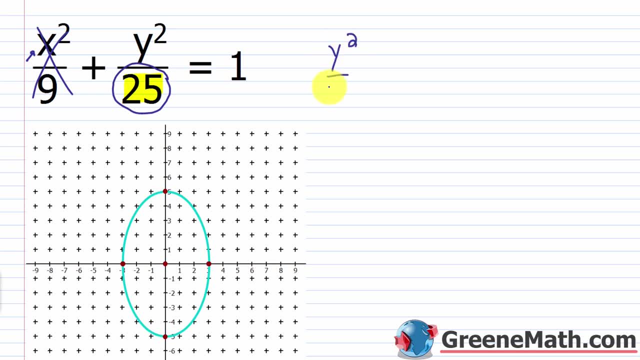 equals 1.. That's easy to solve: y squared over 25 equals 1.. I can multiply both sides of the equation by 25 and get y squared equals 25.. Then I'll take the square root of this side and then plus or minus the square root of this side. So y is equal to plus or minus. 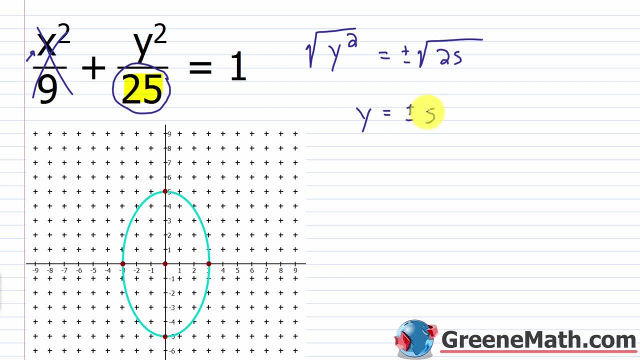 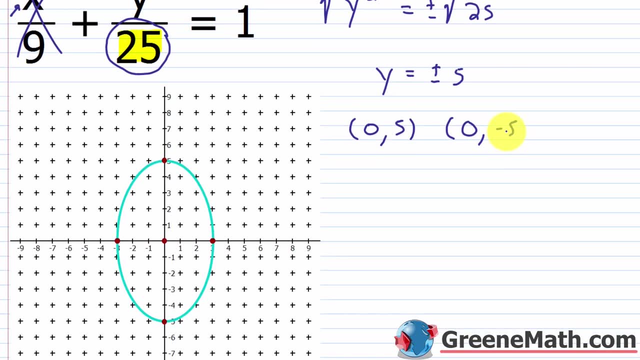 5.. Now with the y-intercept we know that x is 0. So that's what leads to the points 0 comma 5 and 0 comma negative 5.. Okay, those are right here. With the x-intercepts I would do the same thing. 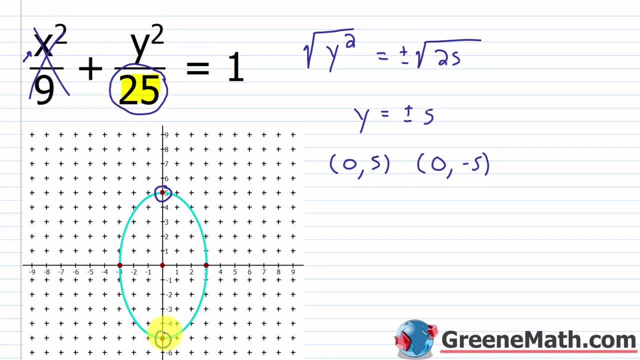 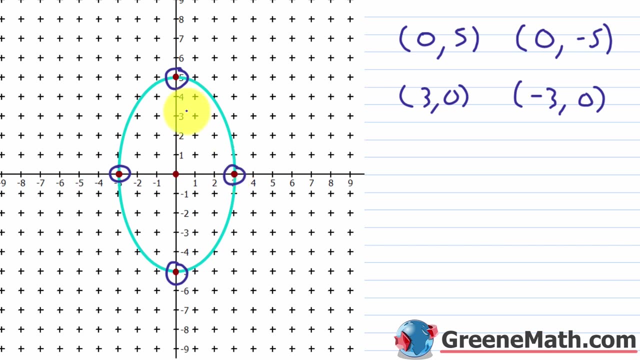 I would just plug in a 0 for y and I would solve for x. You'll find that you would get 3 comma 0 and you would get negative 3 comma 0. So here. so what's creating this shape is the fact that the distance from the center to this 5 up here. 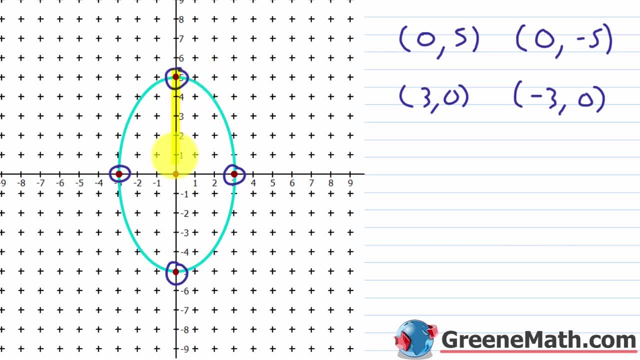 this is 5 units. This, right here, is 5 units. Then your distance from this guy right here to here, Well, this is only 3 units. This is only 3 units. The fact that when we graph this guy, we're drawing a curve through these points, We have to. 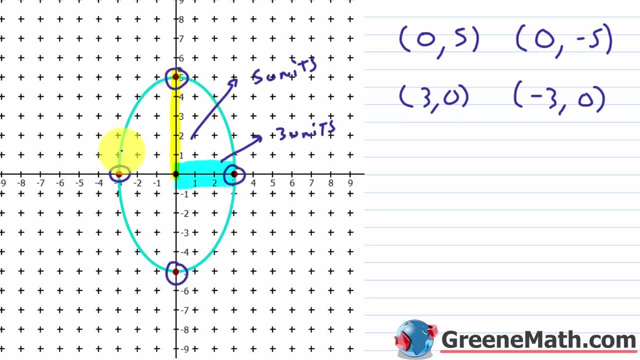 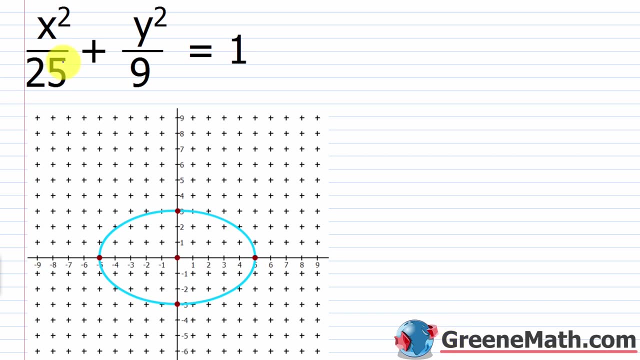 take into account the fact that we have to split this by a half, but in our final» Let's go to next, When we shift from the top of the curve to the bottom of the curve, And let's just take a look To the right. 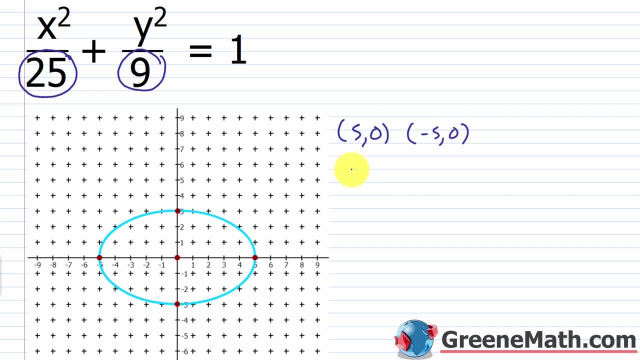 to the right, To the left is exactly the same, To the right is exactly the same. We just deal with this into 9 plus 0, 0 and 0, 7.. and negative 5 comma 0.. The y-intercepts would be at 0 comma 3 and 0 comma negative 3.. So this: 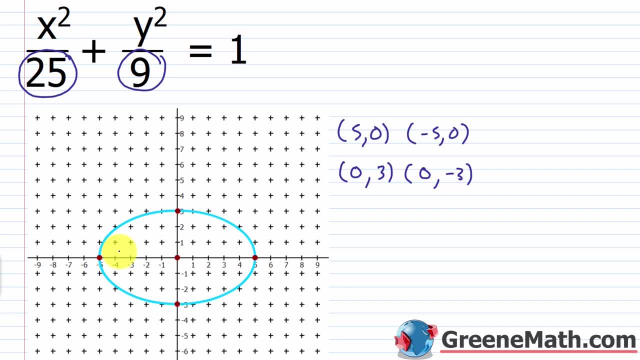 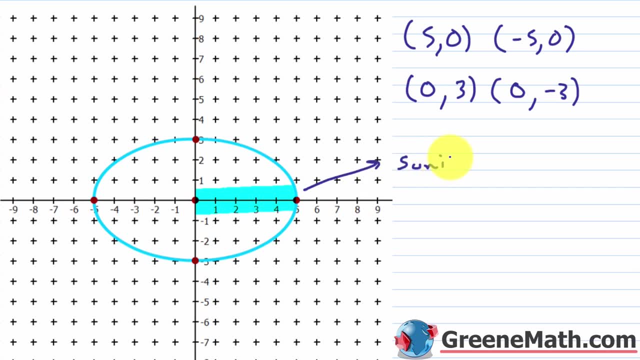 guy changed from being tall and skinny to short and fat. In other words, the distance from here to here is now 5 units, whereas the distance from here to here is now only 3 units. So as this guy gets graphed again, we draw our curve. It's a further distance horizontally when this curve is. 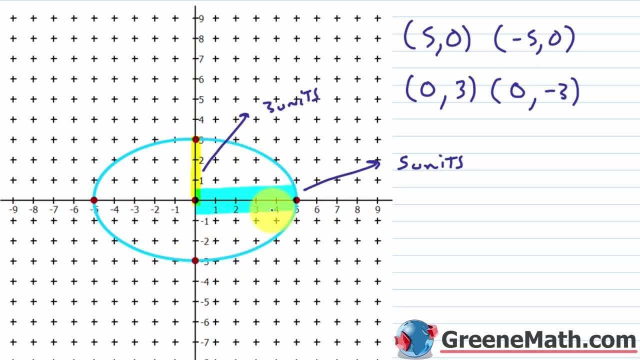 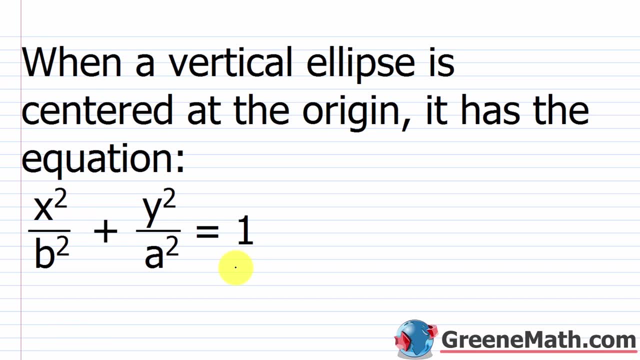 being drawn than it is vertically right, So it creates this shape of being short and fat. So when you start working with ellipses, you're going to see two different standard forms. This can be a little bit confusing at first, but it's something you will get used to When a vertical ellipse is. 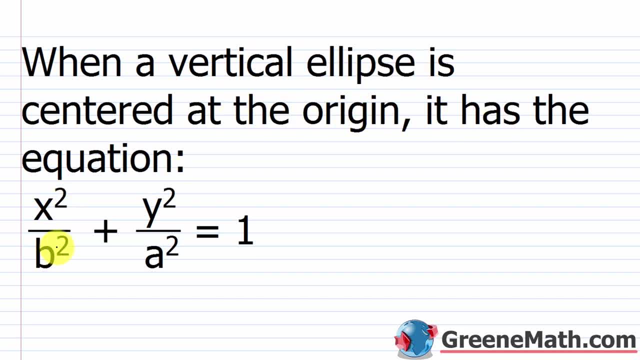 centered at the origin. it has the equation: x squared over b squared plus y squared over a squared equals 1.. Now we talked about the fact that a vertical ellipse has a bigger value here, underneath y squared, than here, And the reason for that is we always want to have a being greater than b. 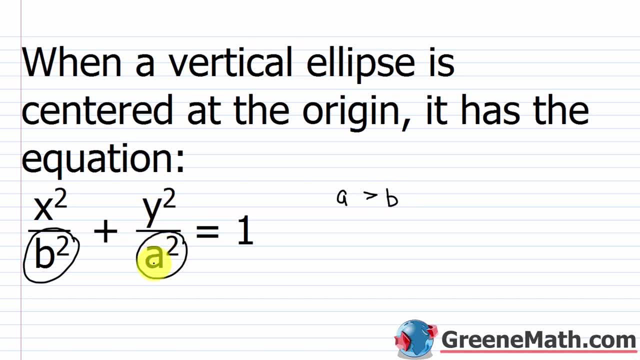 okay. So if the denominator under y- squared, is bigger, you're going to use this formula here. This is for a vertical ellipse, In the case where we have a horizontal ellipse. well, when a horizontal ellipse is centered at the origin, it has the equation x squared over b squared over a squared. So when a horizontal ellipse is, 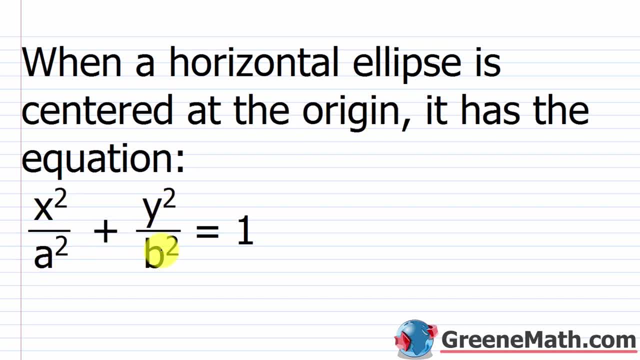 centered at the origin. it has the equation: x squared over a squared plus y squared over b squared equals 1.. In this case we said with a horizontal ellipse, this is greater than this. Again, you've got to set this up to where a is greater than b. This has to do with a formula. 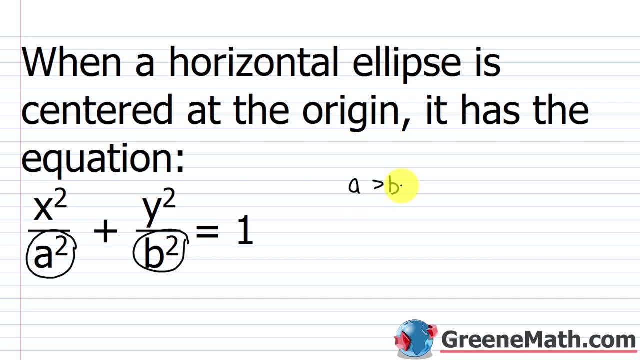 you're going to deal with down the road. When you really start talking about ellipses, you're going to see, for the purposes of subtraction, a is going to need to be greater than b, So that's why these formulas are going to kind of switch back and forth. All right, so how do we graph an ellipse? 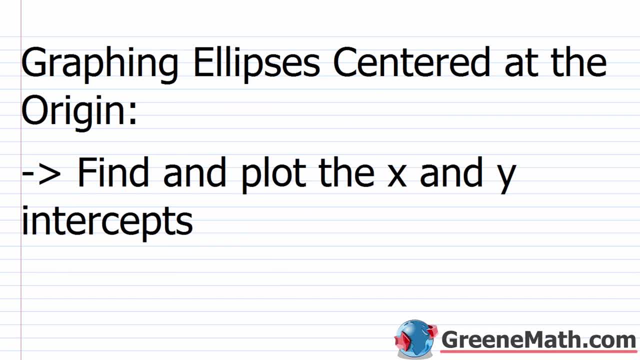 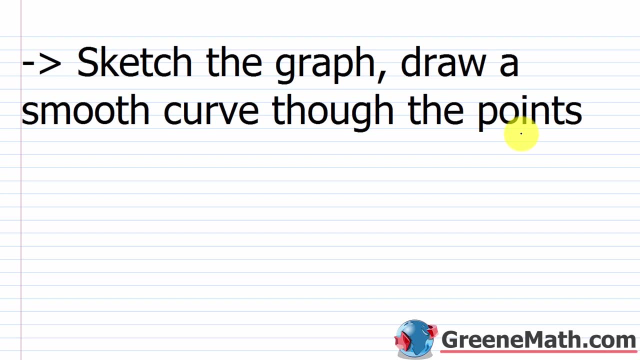 Let's start out with the easy scenario where it's centered at the origin. So we have graphing ellipses centered at the origin. We first want to find and plot the x and y intercepts. Then we just sketch the graph, draw a smooth curve through the points. So just like we saw when we graphed a 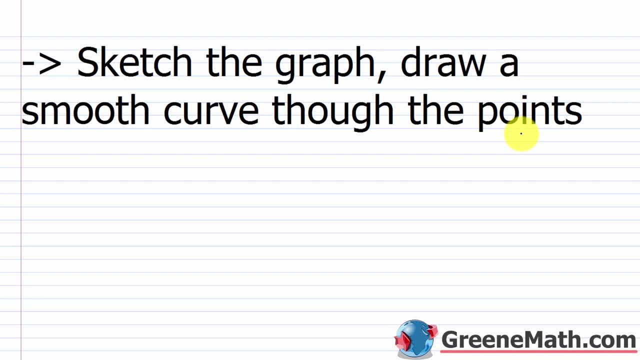 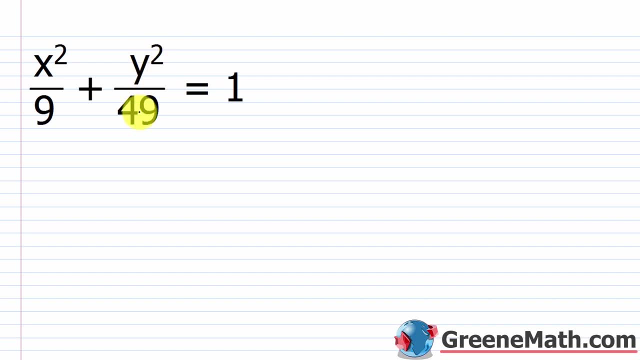 circle, we'll end up with four points and we just draw a smooth curve through the points. All right, so let's start out with this first example. We have x squared over 9, plus y squared over 49, and this equals 1.. 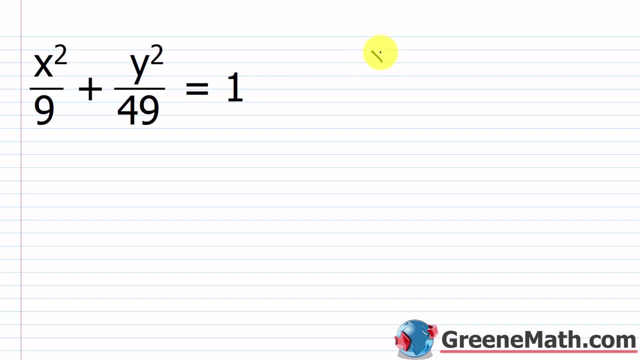 So the first thing is: how do we find our x intercepts- And let me make that a little better- And how do we find our y intercepts? Well, this concept has not changed from when we first learned it, when we were working with linear equations and two variables. Essentially, if I want the x to be greater than b, I'm going to have to find the x squared over 9 plus y squared over 49.. So the first thing is, how do we find our x intercepts? And let me make that a little better. 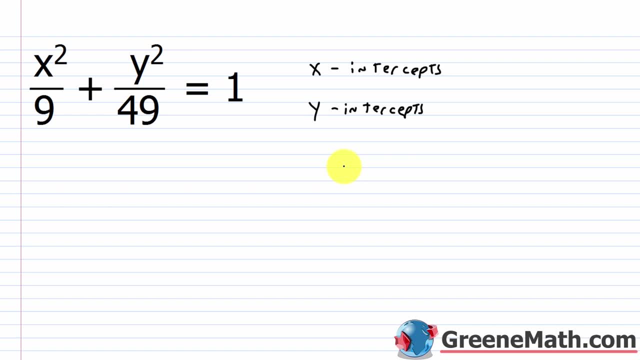 I want to make y equal to 0, and I want to solve for x. So I know that it's something. comma 0 in each case, right, because y is 0.. So if this is 0, this is gone right. 0 squared is 0, 0 over 49 is. 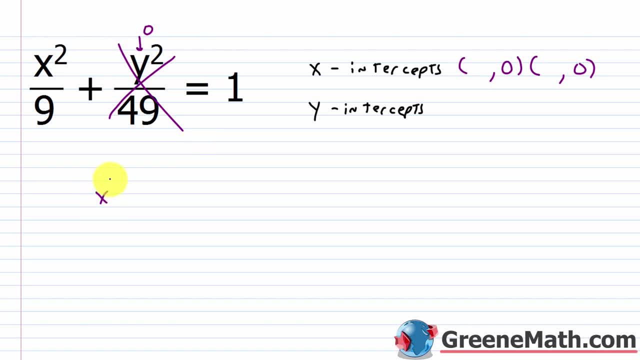 0.. It's gone. So we have x squared over 9 is equal to 1.. I multiply both sides of the equation by 9, and we know that this would cancel with this, and I have x squared is equal to 9.. Now to solve this. 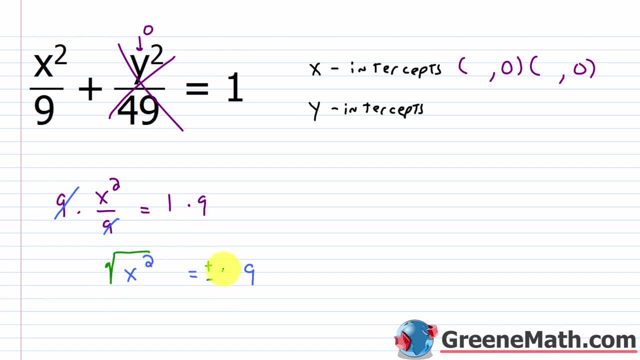 for x. I take the square root of this side. I take plus or minus the square root of this side and I get that x is equal to plus or minus 3.. So the x values when y is 0 would be positive. 3. 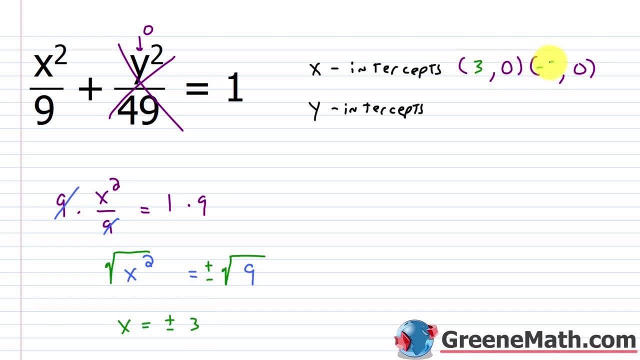 and negative 3.. Now, what's the shortcut here? Because I don't need to go through this every single time. What ends up happening is if this guy right here is a 1, which is always going to be in the case of an ellipse sometimes. 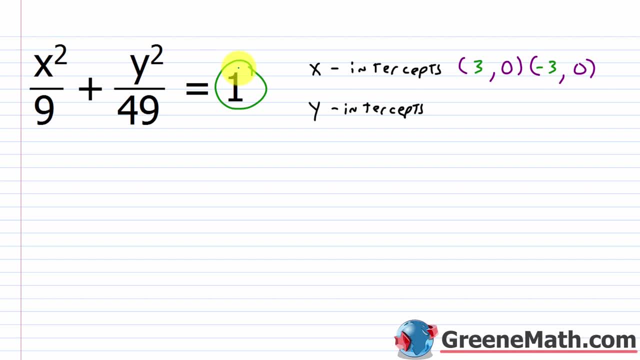 you'll get an equation that you have to put into this form. but once it's put into this form, this is what you're going to see. So what happens is, if this is always gone, let's just say: this is x squared over q. Doesn't matter what q is, it's just a placeholder for now, and this equals: 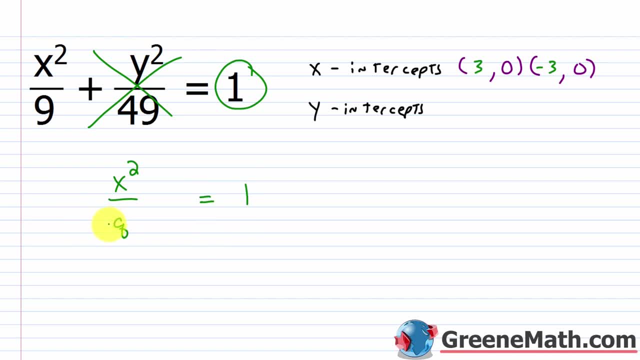 1. Well, I'm always going to multiply both sides of the equation by q, So I'll have x squared equals q. And to solve this I'm going to take the principal and negative square root of q every time right, So x would equal the positive and negative square root of q. So to get the x values, 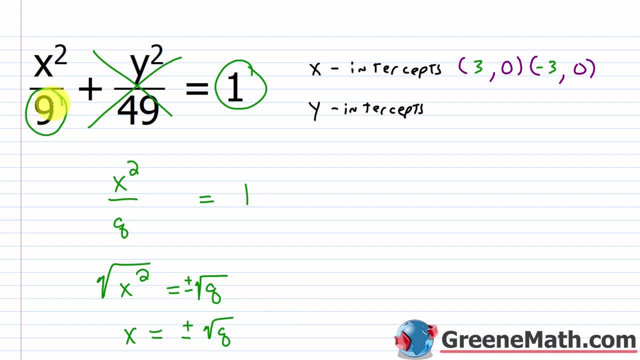 for the x-intercept. I just need to look at this denominator here and take the principal and the negative square root of that. I don't need to go through plugging in 0 and doing all this work, because in every situation that's what's going to happen. 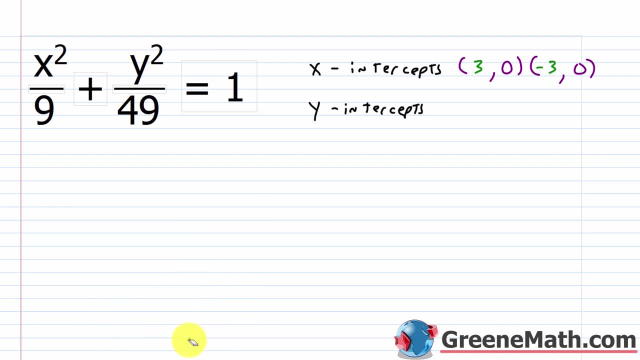 Same thing goes for finding the y values for the y-intercepts. I already know that the x values are 0. I don't need to guess on that. So if I went through the whole thing, I'd plug in a 0 there. 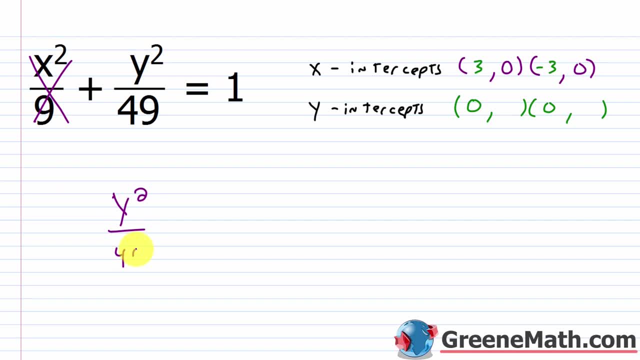 This would be gone. I have y squared over 49 equals 1.. I multiply both sides of the equation by 49. That cancels. I get y squared is equal to 49.. Again, I take the square root of this side. 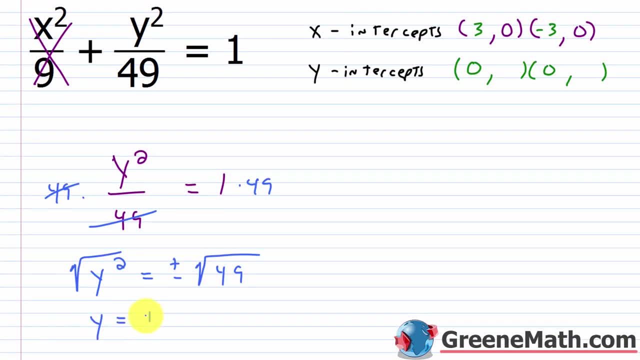 or minus the square root of this side. So we get: y is equal to plus or minus 7.. So 0 comma 7 and then 0 comma negative 7.. But again, the shortcut would be to just take this guy right here and say: 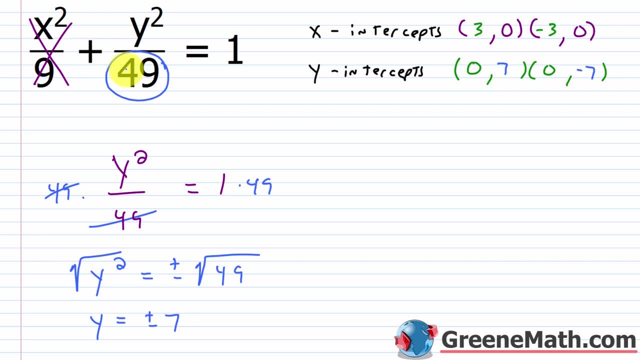 OK, for the y values. for my y-intercepts I just take the principal and the negative square root and that's how I get them right. Positive or negative square root of 49 would be plus or minus 7.. So once we have the intercepts, the process is very, very easy. It's just like graphing a. 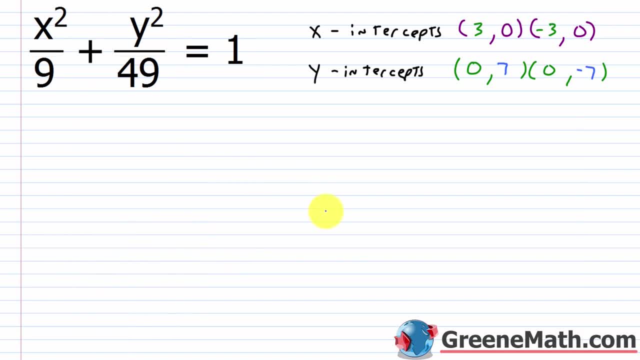 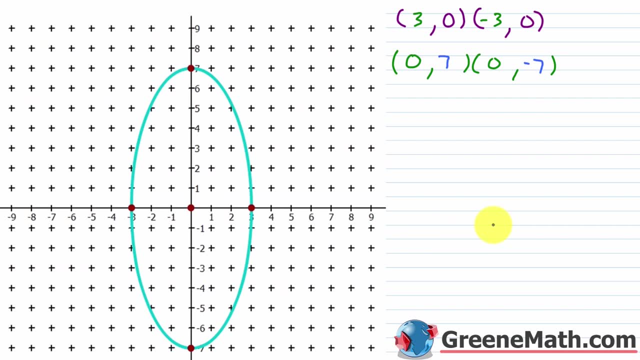 circle. We just plot the points and then we sketch a smooth curve through the points. So let's take these points down to the coordinate plane, All right? So we have everything kind of pre-drawn, just to make it a lot easier for us. So here's: 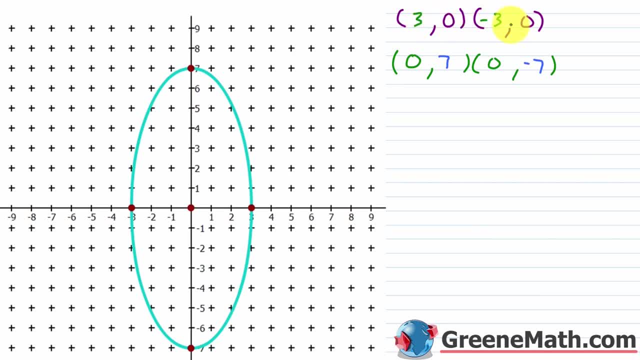 our points. We have the x-intercepts that occur at 3 comma 0 and negative 3 comma 0. So here's 3 comma 0 here, Here's negative 3 comma 0. So those are two points. Then my y-intercepts occur. 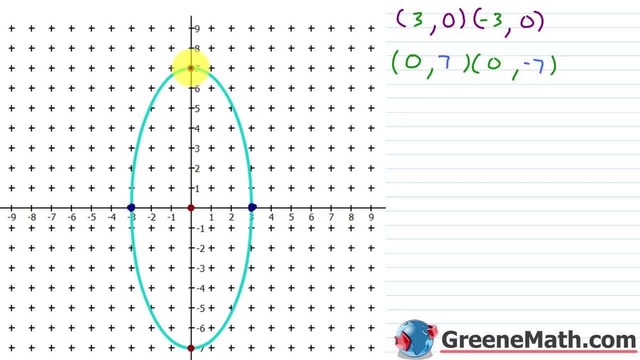 at 0 comma 7 and 0 comma negative 7.. So here's 0 comma 7, and here's 0 comma negative 7.. And then I just need to sketch the curve around those points So you can see the computer did a. 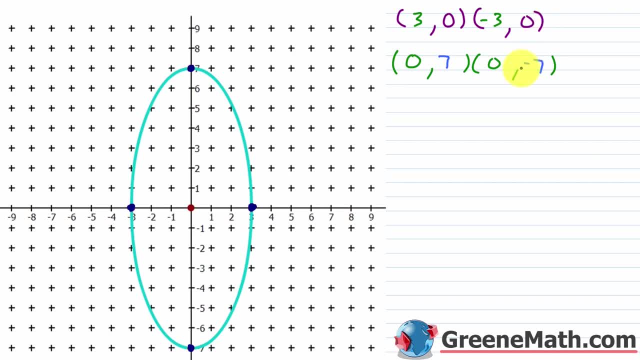 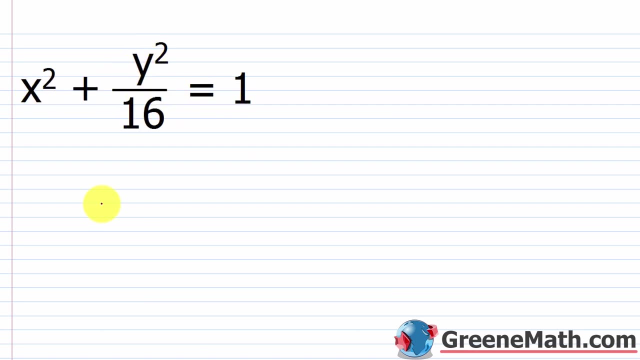 perfect job. I'm going to trace over what they did and I will attempt to do a mediocre job. All right, Let's take a look at another one. So we have x squared plus y squared over 16 equals 1.. So the first thing is, if I don't have a visible denominator under x squared or y squared, 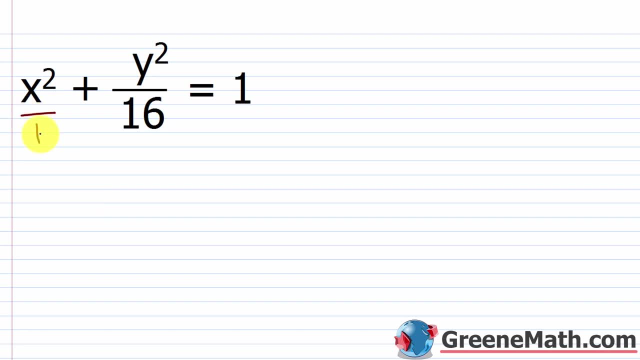 I'm going to put this guy y over 1.. The reason for that is I'm going to need to use these denominators to again get my x and y-intercepts. So for the x-intercepts again, we learned the shortcut for that. 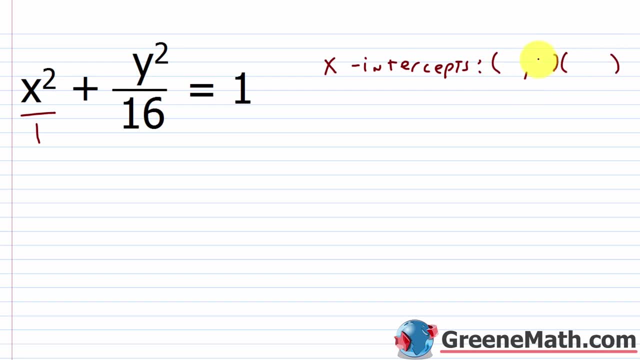 So they would occur where We know the y values are 0 in each case. What are the x values? Again, I look at this denominator under x squared. I take the y-intercepts and I'm going to use the x-intercepts. So I'm going to use the x-intercepts. 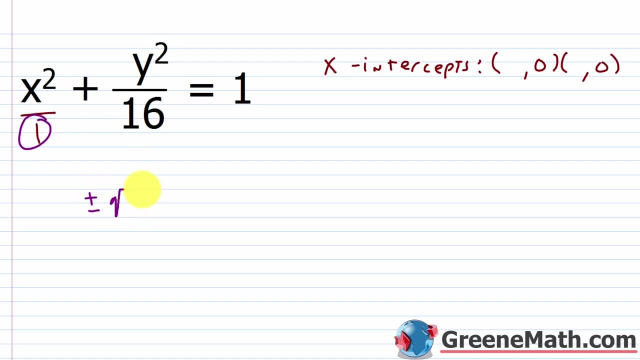 to get the principal and negative square root of that. So, plus or minus, the square root of 1 is plus or minus 1.. So I get positive 1 and negative 1 as my x values. Then for the y-intercepts we would get what? Well, we know that the x values would be 0 in each case. And again, 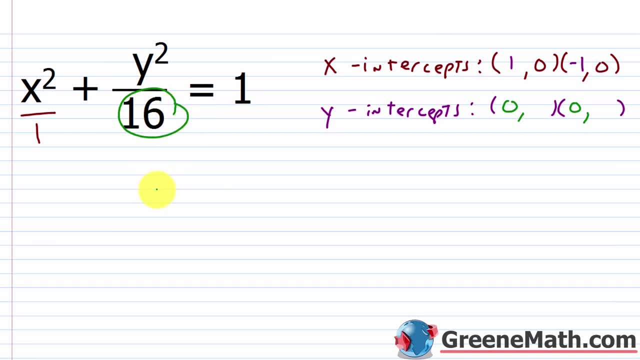 I would just look at my denominator here. In this case it's 16.. I take the principal and negative square root of that, So plus or minus the square root of 1 is plus or minus 1.. So I get negative square root of that guy. This equals plus or minus 4.. And so the y values here would be 4. 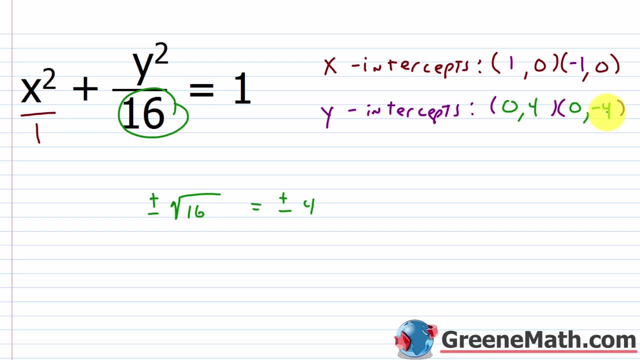 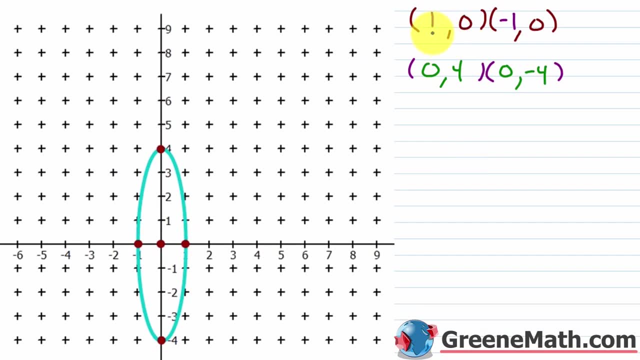 and a negative 4.. So again, very, very easy to get these points going: I just take them down to the coordinate plane. now, All right, So we would start out by plotting the point 1, 0.. So 1, 0 is here. 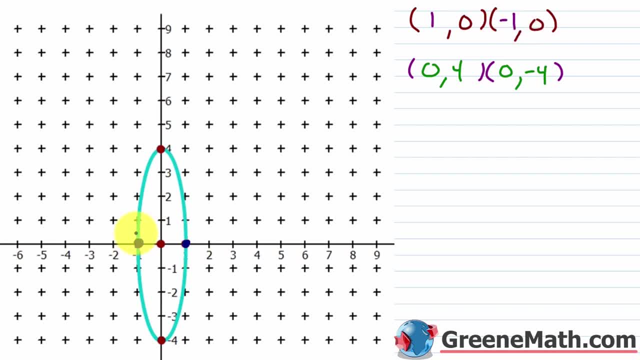 And then negative 1, 0 is here, And then 0, 4 is here, And then 0, negative 4 is here. So we have our intercepts plotted And then again we're just going to graph a smooth curve through the. 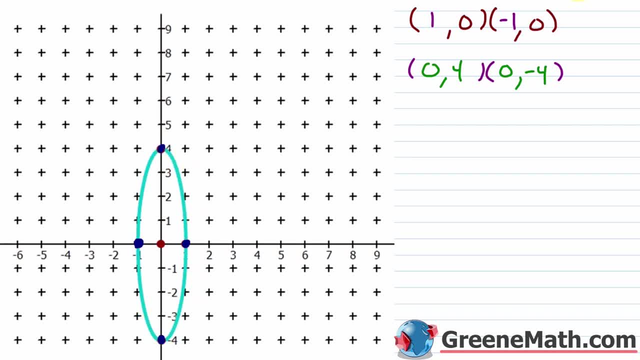 points. Again, the computer did a perfect job already, And I am going to again attempt to do a mediocre job by tracing over what the computer did, So let's go ahead and do that. Okay, So again, not perfect, but you get the general idea of what this guy would look like. 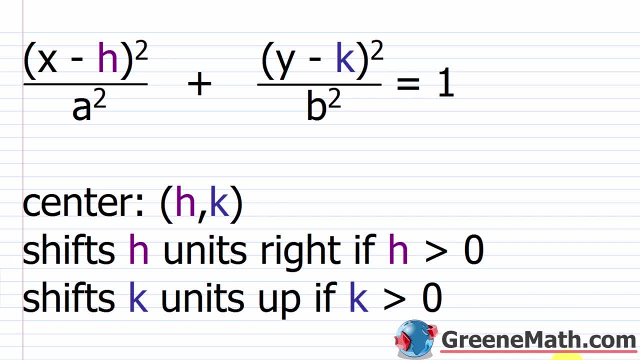 And that's what you're looking to do. So, just like when we saw circles that weren't centered at the origin, you're also going to see ellipses That aren't centered at the origin as well. So, generally speaking- and this will change up- 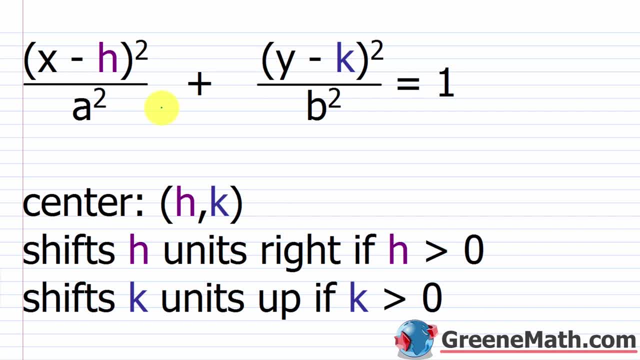 based on if you have a horizontal ellipse or a vertical ellipse. but let's just use the formula for a horizontal ellipse just to kind of think about this. We have the quantity X minus H now squared over A squared. Plus we have the quantity Y minus K squared over B squared. This equals 1.. 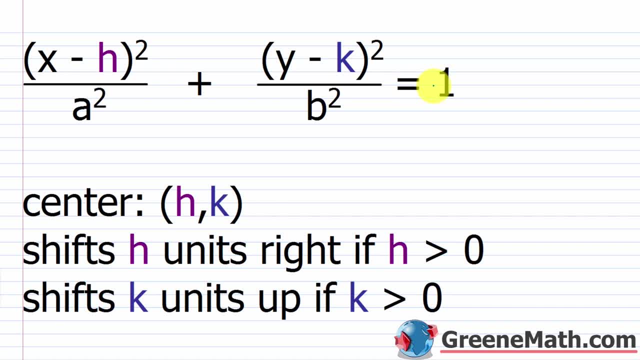 Now, if you had a vertical ellipse, the difference would be that this guy right here would be B squared And this guy right here would be A squared. But again, to keep things simple, let's just work with the horizontal ellipse for right. this second, The center will occur at H. 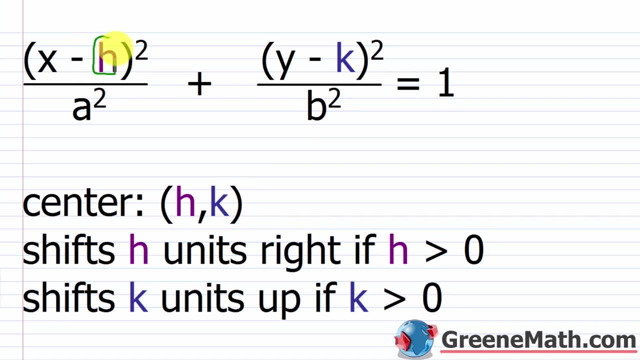 comma K: Okay, So whatever's right here for H and whatever's right here for K, but that's given that you have a minus sign here and a minus sign here. You've got to pay attention to that, because if you end up with a plus something, 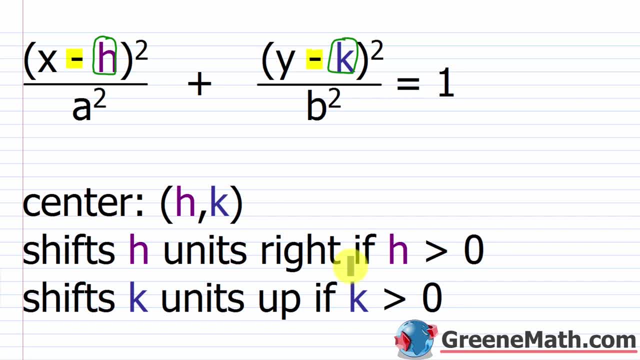 you've got to make an adjustment to match the formula. So what we can say is that this guy shifts H units to the right If H is greater than zero. if H was less than zero, then what would happen is it's shifting H units to the left. Then we can also say: it shifts K units up if K is greater than zero. 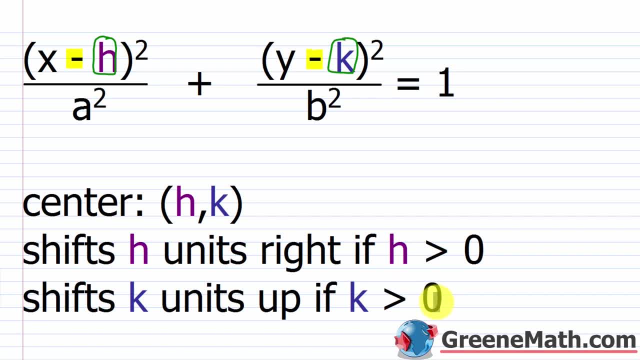 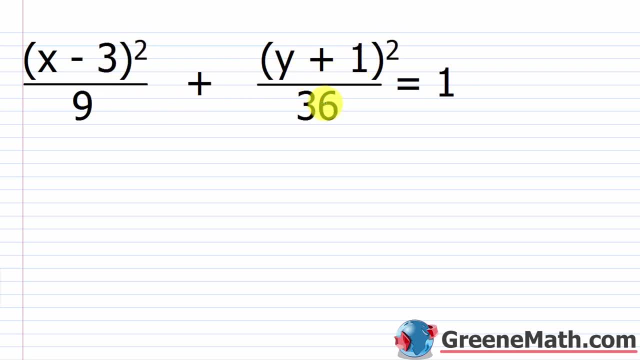 or it would shift K units down if K was less than zero. All right, So let's take a look at X minus three, that quantity squared over nine. Plus, we have Y plus one, that quantity squared over 36.. This equals one. So the first thing is, this guy will be a vertical ellipse. We know that because 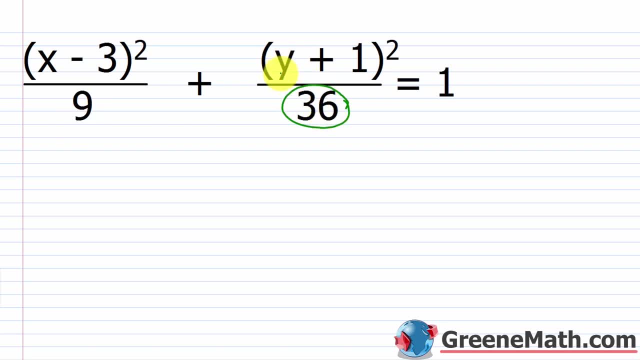 the 36 is larger than the nine, So we can say that this guy will be a vertical ellipse. Now that we've gotten kind of that out of the way, we think about how could we graph this guy? Well, if I was graphing X squared over nine plus Y squared over 36 equals one. 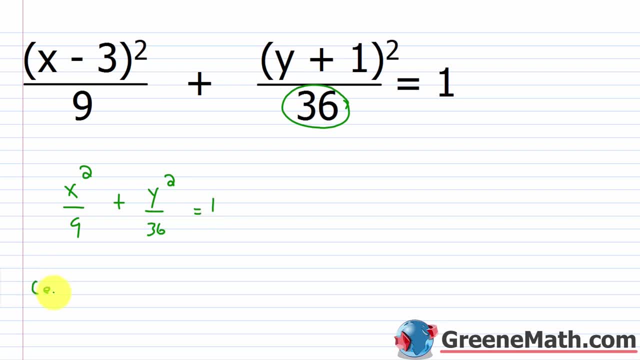 what would I do? Well, I know the center, I know the center is at zero comma zero. I know my X intercepts Are where. Again, I would look at this guy and I would go plus or minus the square root of that. 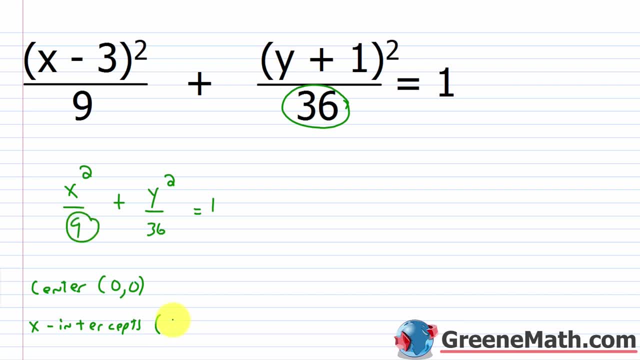 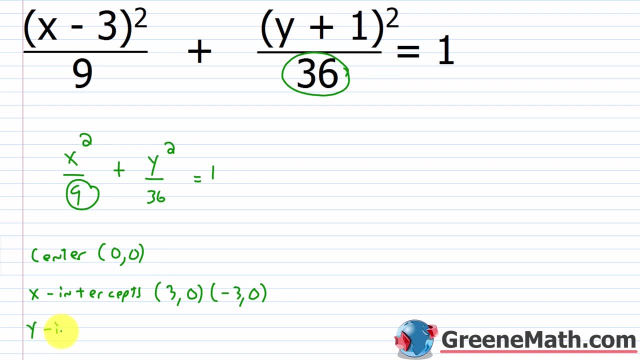 plus or minus, the square root of nine is plus or minus three, So three comma zero, and then negative three comma zero, And then my Y intercepts. my Y intercepts would occur where, Again I'd look at this- plus or minus, the square root of 36 is plus or minus six, So zero comma six. 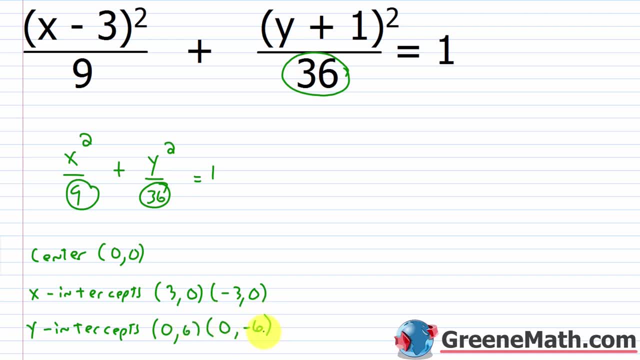 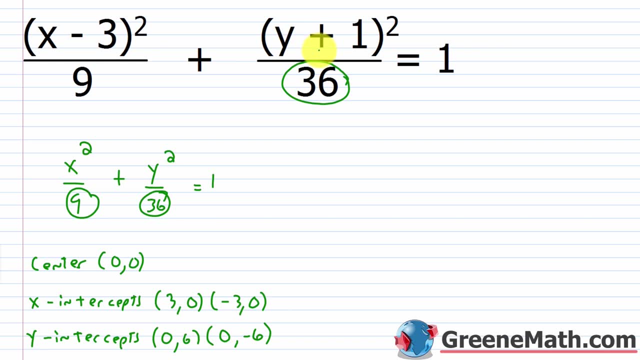 and a zero comma negative six. Okay, So I could plot those four points, I could sketch my curve around the four points and I'd be done. What happens is this guy we're looking at here has been shifted three units to the right and one unit down, So the center. 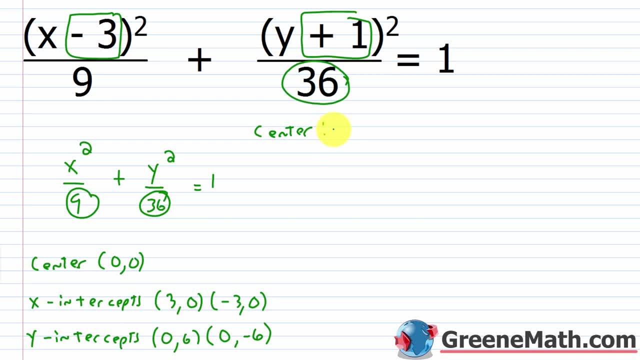 will now be at three comma negative one. You might say: well, where did you get that? Again, the formula is X minus H, that quantity squared over. In this case we have a vertical ellipse, So this would be B squared. But we take whatever's right here after. 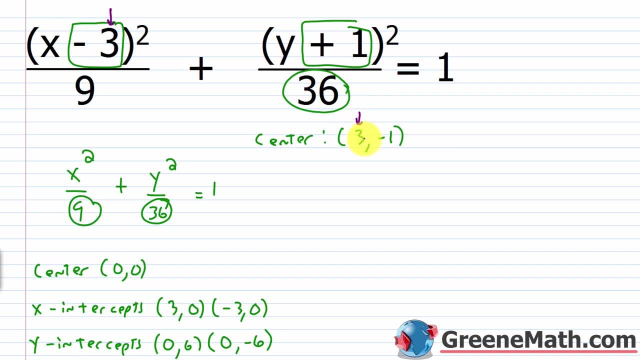 the minus sign. So in this case that's three. That is the X value for the center. Then we have plus, we have Y minus K, that value squared. And then again, because this is a vertical ellipse, this would be A squared here And this equals one. But whatever, this guy right. 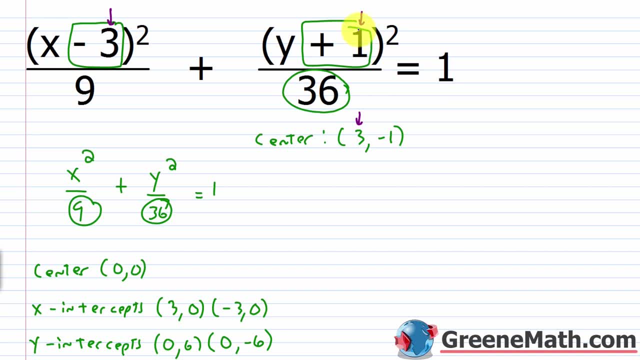 here. if this was minus, we're taking that. Now it's not a minus, I have a plus here, So I want to rewrite this as minus. on negative one, So it matches the formula and I can just take negative one and plug it in as my Y coordinate for the center. So now I know, let me just kind. 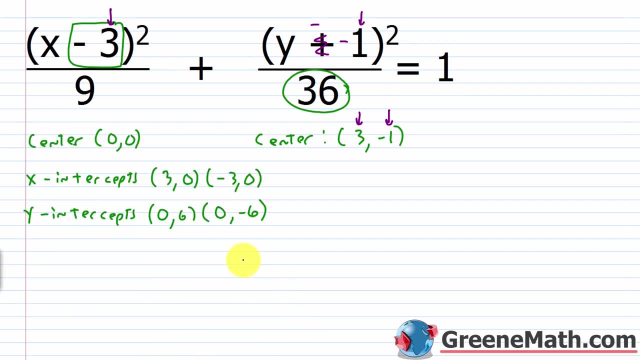 of erase this If I scooch this up. I know that these points here have just shifted three units to the right and one unit down. Now they're no longer the X and Y intercepts, They're just going to be two points. Every time I took the Y intercepts they just became the furthest points. 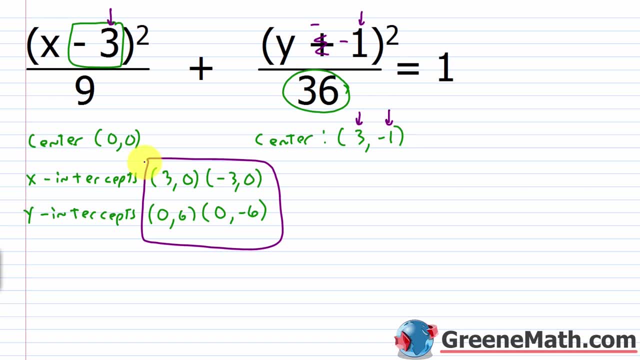 to the right and to the left of the center on the ellipse For the Y intercepts it's the furthest point above the center and below the center on the ellipse. So these are just four additional points we're going to get. So if I take three comma zero and I shift it three units to the 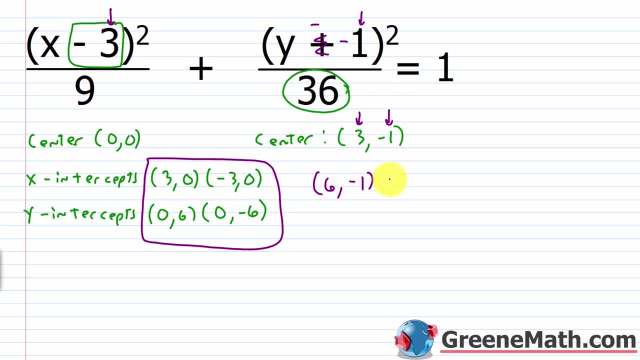 right and one unit down, then I would get six comma negative one. If I take negative three comma zero and I shifted it, three- see the right- and one unit down. Yeah, zero, Shelly, extremely. So people believe we're gonna get 3,380!. 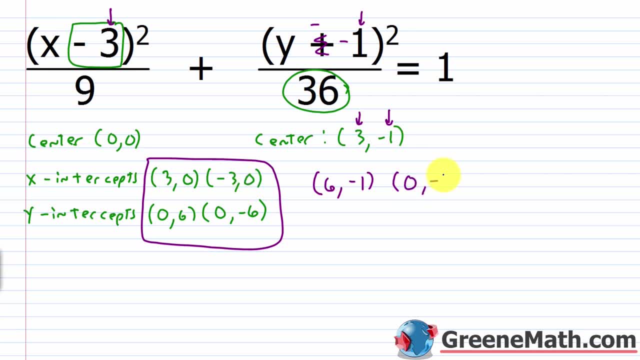 unit down, I would get 0, negative 1.. If I take 0, 6, and again I shift it 3 units to the right and 1 unit down, I would get 3, 5.. And lastly, if I take 0, negative 6, and I shift it 3 units to, 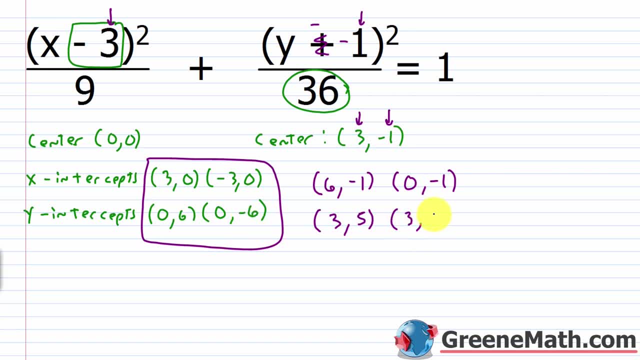 the right and 1 unit down, I would get 3, negative 7.. Now each time I do this, I don't want to go through this comparison. So the easy way to kind of do this is to just find the center based on the. 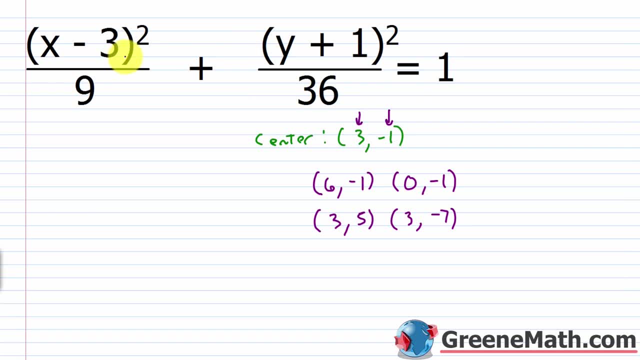 formula. We know we're looking for h, k. We know how to find those values. That's my center. For points where we move horizontally from the center, I'm looking at this value here. So plus or minus the square root of that would be the horizontal distance from the center. again to the furthest. 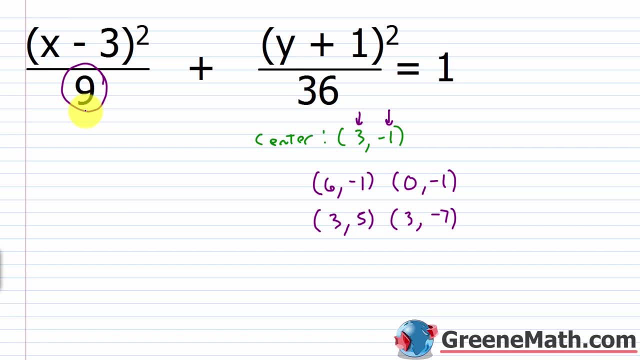 point to the right and to the left on that ellipse. So starting at 3, negative 1, I could add the center to the center. So I'm going to go through this comparison. So the easy way to kind 3 to my x value and get 6, negative 1.. And I could subtract 3 from my x value and get 0,. 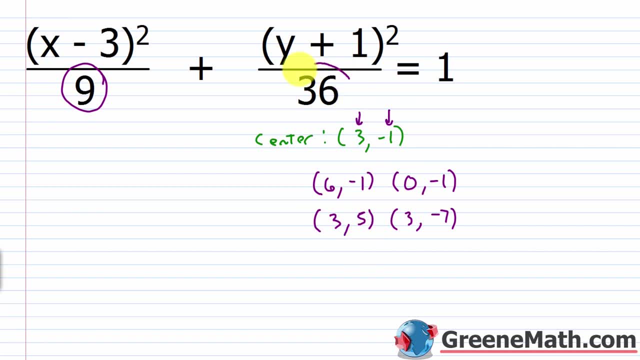 negative 1. There's two points there. Then I take this guy right here, And now I'm thinking about getting a vertical distance from the center to the highest and the lowest point on the ellipse. Then plus or minus the square root of 36 would give me that. So that'd be plus or minus 6.. 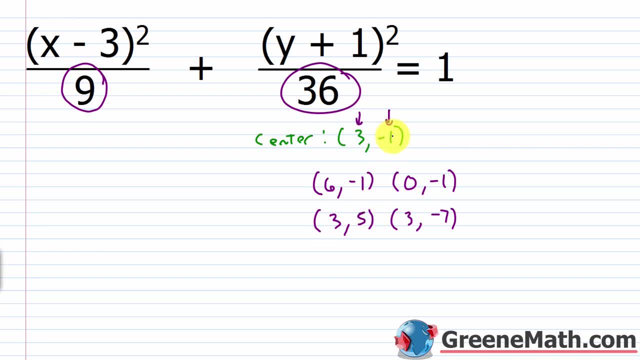 With negative 1, I go up by 6, I get to 5.. With negative 1, I go down by 6, I get to 5.. So that's how you could quickly get those four points. You grab the points. Let's start out with. 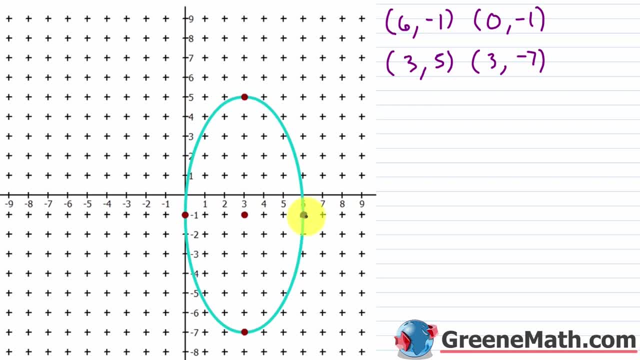 6, negative 1.. So that's going to be right here. We would have 0, negative 1,, which is right here. So again, from the center, this is moving 1, 2, 3 units to the right and 1, 2, 3 units to the left. 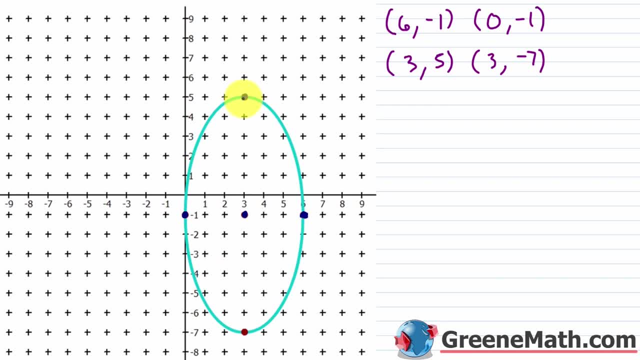 Then we have 3, 5.. So that's right here. And then we have 3, negative 7.. That's right here. Right here Again, from the center, I'm moving 1,, 2,, 3,, 4, 5, 6 units up and 1,, 2,, 3,, 4,, 5, 6 units. 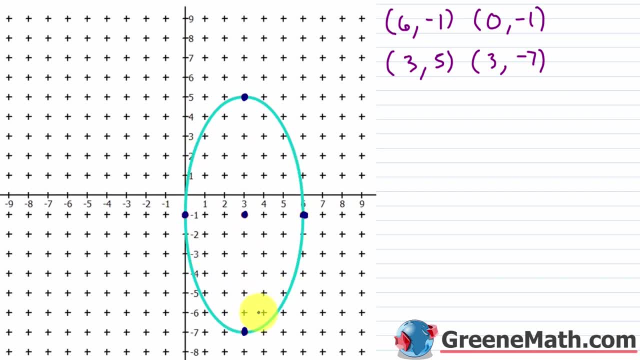 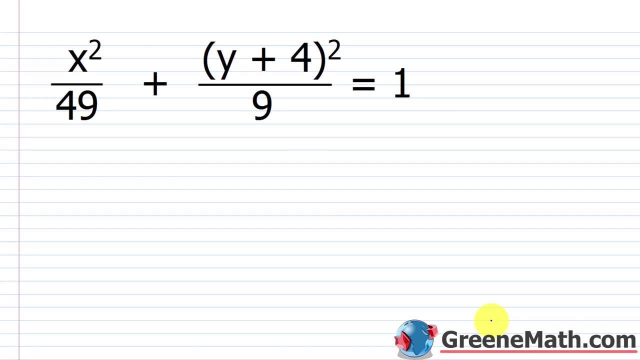 down. So that's how we would get my four points, And again, I'm just going to draw a smooth curve through the points. Okay, Again, not perfect, but you get the general idea of what this guy would look like. All right, Let's take a look at one final problem now. So we have x squared over 49. 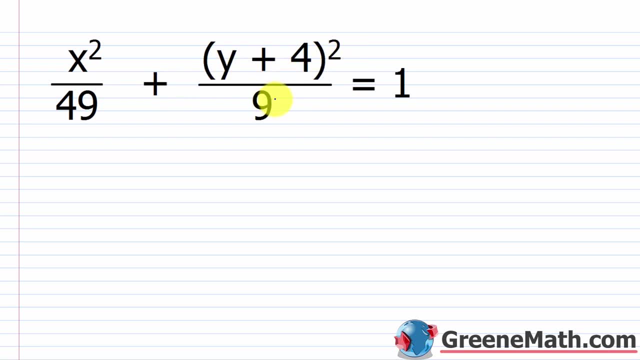 plus, you have the square root of 36.. So that's right here, And then I'm just going to draw a y plus 4 squared over 9. This equals 1.. So this guy, we want to start by again finding the. 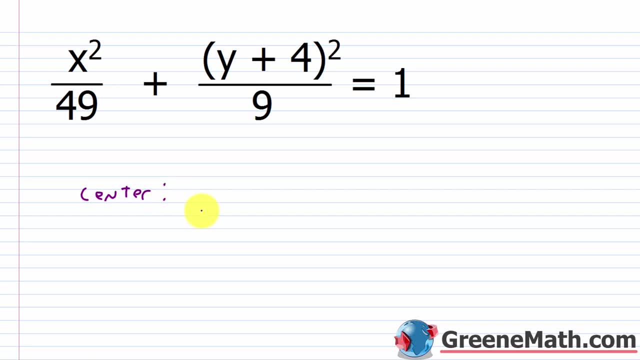 center, And in this case we have what? The 49 is bigger than the 9.. So this would be a horizontal ellipse. So the center occurs where It's, at h comma k. I just have x squared here, I don't. 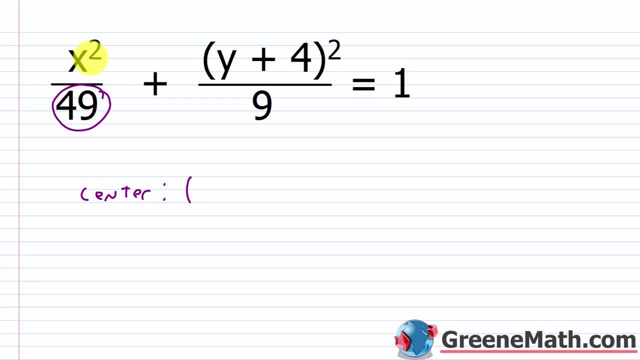 have x minus something. I don't have x plus something. That quantity, I don't have that squared. So I'm just going to draw a smooth curve through the points And then I'm just going to the center. will occur here: The x value hasn't shifted, It's just 0.. And to really write this in: 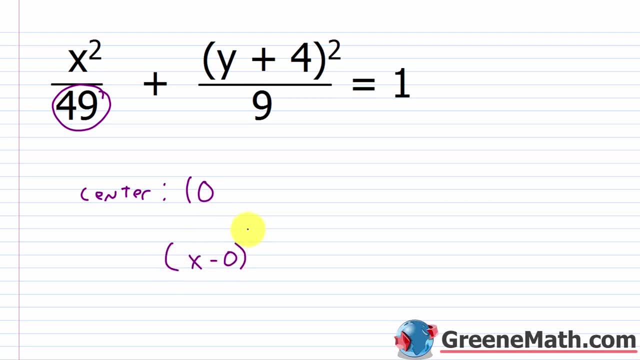 that format, you could say this is x minus 0.. That quantity squared over 49.. So this guy right here is your x value, which is 0.. Now for the y value. again, I want to write this as minus a negative 4.. 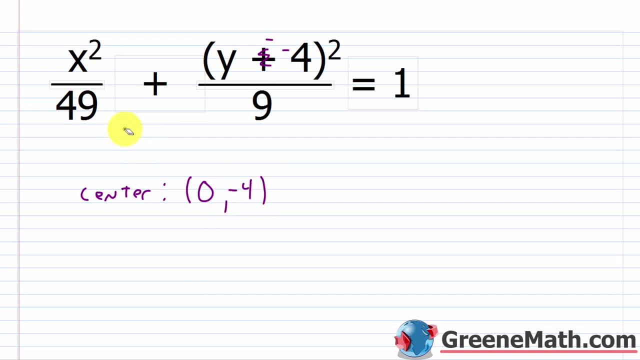 So negative 4 would be the y value there. And then to get my additional points again, all I'm going to do is take some horizontal points from the center. I just take this guy right here. I take the principal negative square root of it. Principal negative square root of 49 is 7.. So I'm just going. 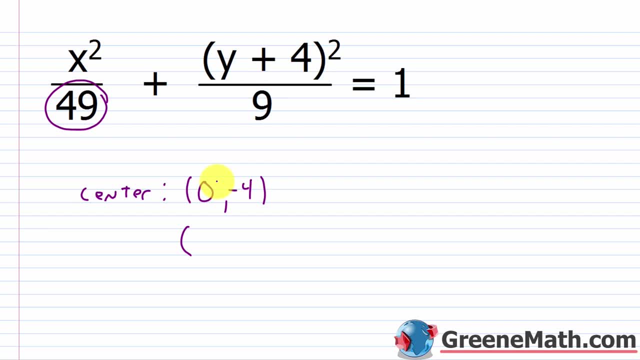 to move by 7 units to the right of the center and to the left of the center. So add 7 to 0, you get 7, then comma negative 4.. Subtract 7 from 0, you get negative 7, comma negative 4.. Then over here. 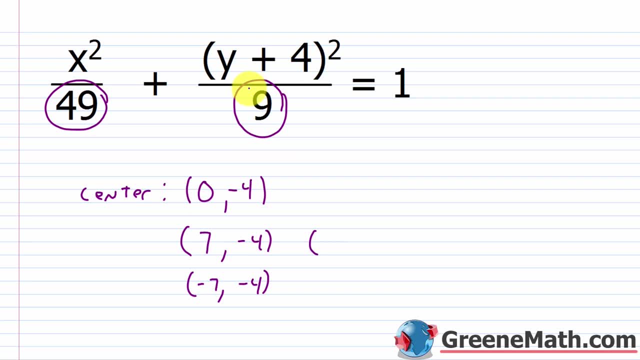 again, I'm going to do the same thing for this guy: Plus or minus. the square root of 9 would be plus or minus 3.. So from the center, I'm now going to look for points that are vertically above the center and below the center. So my x value stays. 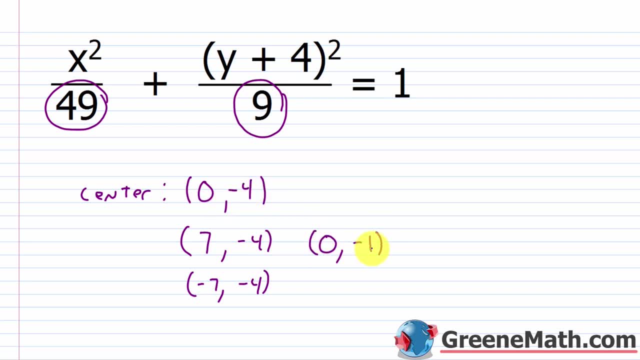 the same: Negative: 4 plus 3 would be negative 1.. And then again, my x value stays the same: Negative: 4 minus 3 would be negative 7.. So there's your four points there. So again, 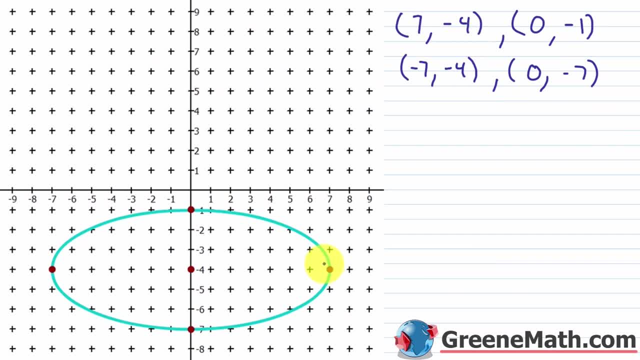 we're going to plot these four points. You have 7 comma, negative 4.. That's right here. And you have negative 7 comma, negative 4.. So that's right here. Again, in each case, from the center, we just moved 7 units to the right and 7 units to the left. Okay, So that's how we got. 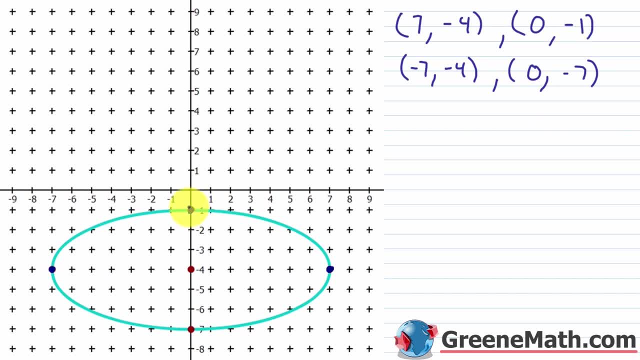 there. Then we have 0 comma negative 1. And we have 0 comma negative 7. Again from the center, we moved 3 units up and 3 units down. So let's go ahead and sketch the graph here. 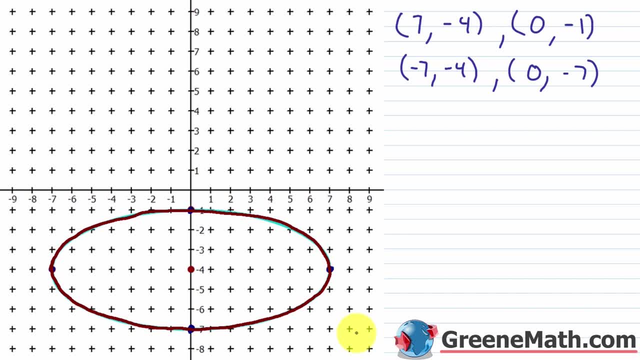 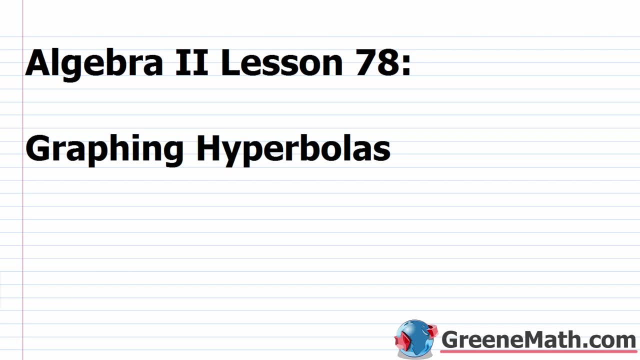 Okay. So again, not perfect, But again just giving a general idea of what the ellipse would look like. Hello and welcome to Algebra 2, Lesson 78.. In this lesson we're going to learn about graphing hyperbolas. So up to this point, we've learned how to graph parabolas, how to graph circles. 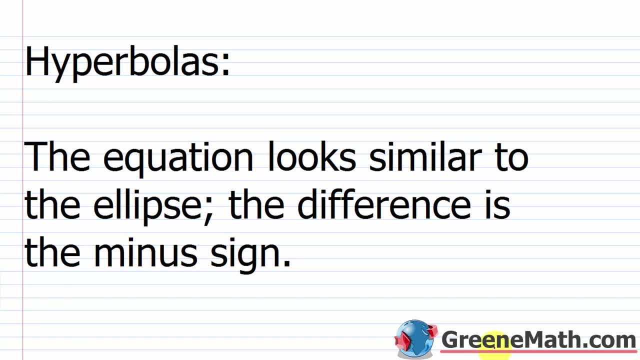 and how to graph ellipses. So the next thing we're going to come across is how to graph the hyperbola. So these are a little bit more challenging to draw. But again, when you're working with these things, especially if you're freehand drawing something, the expectation is: 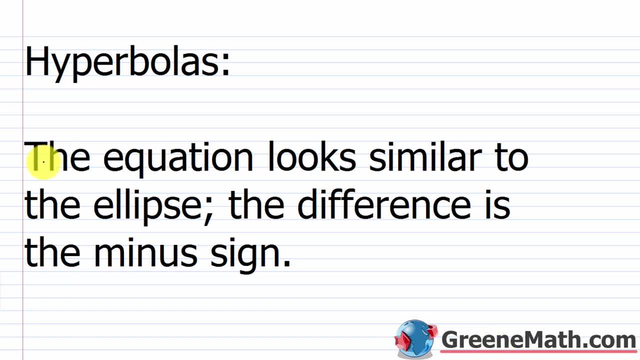 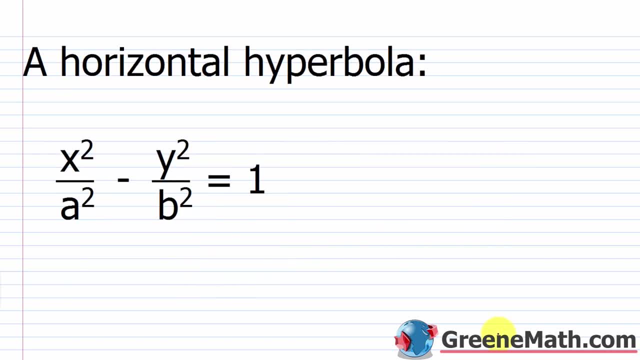 to have a general idea of what it looks like. So with hyperbolas, the equation looks similar to the ellipse. The difference is the minus sign. So I want you to recall that when you worked with ellipses, you had a horizontal ellipse that was short and fat And you had a. 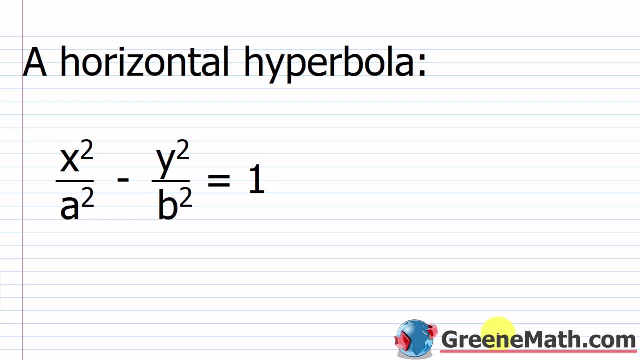 vertical ellipse. that was tall and skinny. When we look at hyperbolas, you're going to have two different scenarios that occur. You'll have a horizontal hyperbola and you'll have a vertical hyperbola. So, with a horizontal hyperbola, you get this equation in your textbook. You'll see x squared. 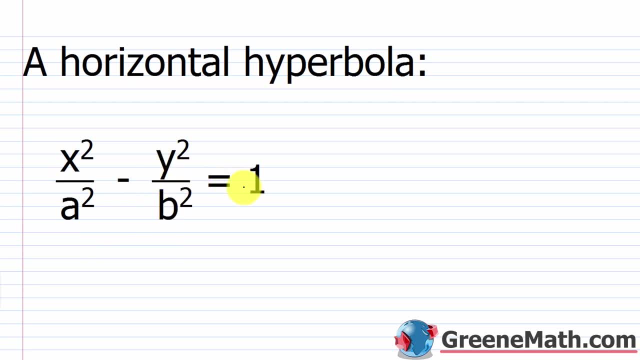 over a squared, minus y squared over b squared equals one. Now let's stop for a minute. Let's go back to when we learned about ellipses. The horizontal ellipse had the following equation: It was x squared over a squared plus, it was y squared over a squared and it was x squared over a squared. 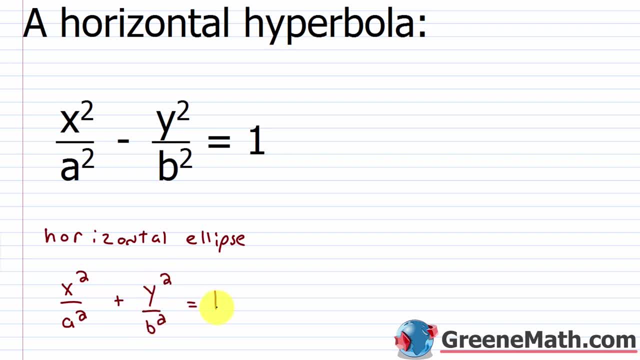 So it was y squared over b squared and this was equal to one. The difference between this equation and this equation is the minus sign here. That's how you know that you have a hyperbola versus an ellipse. Once you figure that out, you have to be able to establish: do I have a horizontal? 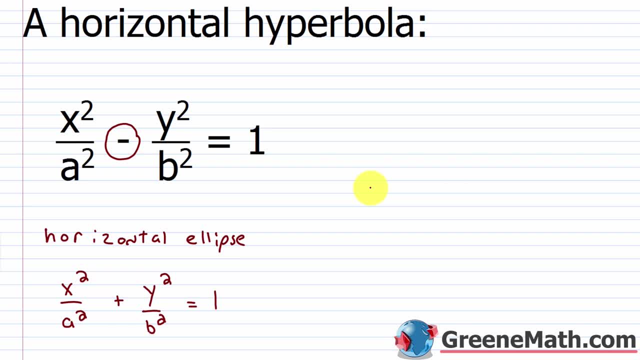 hyperbola Do? I have a vertical hyperbola, And this comes from looking at which term is positive and which term is negative. So in other words, I can think about this term right here. I can say: this is plus negative, y squared over b squared. So if this term is negative, 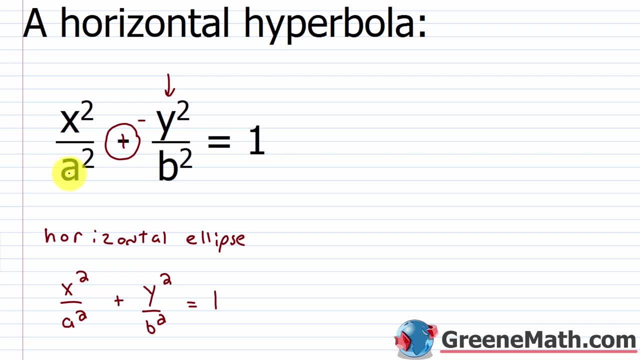 the term. that's positive. if that contains the x variable, we're going to have a horizontal hyperbola. Again, think about the x-axis as being the horizontal axis, the y-axis as being the vertical axis. So in this case, you can think about it as. let's go back to the original. 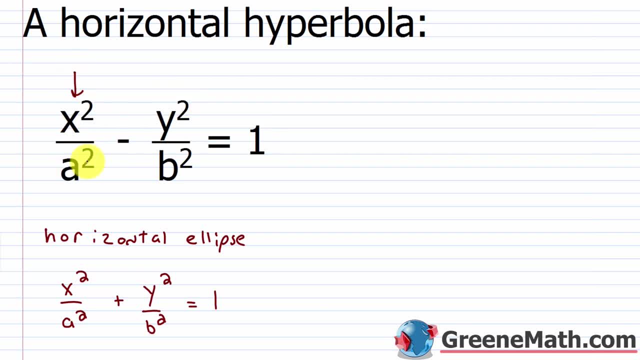 this guy- right here, the x squared over a squared- is larger or more dominant than this guy right here, the y squared over b squared. You might say, well, how do you know that This guy minus this guy equals this guy? If this guy minus this guy equals one, one is a positive number. So 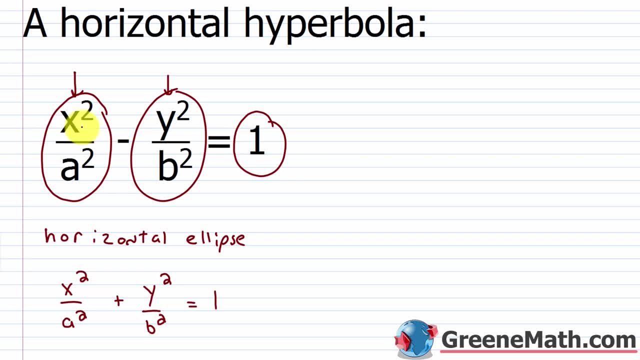 for that to be true, whatever I started with, the x squared over a squared had to be larger than y squared over b squared, because I've got a positive amount left. Just think about if you're spending money out of your checking account, If the result of paying a bill leaves your checking. 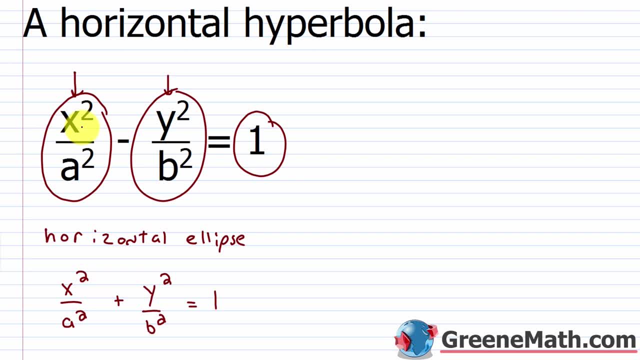 account, a positive balance. well, the bill was smaller than what you started with, So it's the same thought process here. So, however, you want to remember that, if you want to think about the fact that this term is bigger than this term, or you want to say, well, this x squared over a squared. 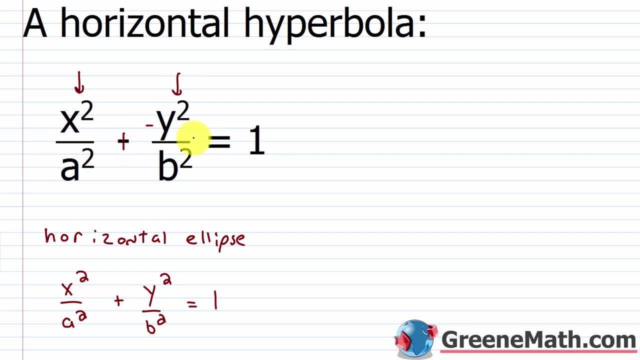 is positive and this guy is negative. however, you remember it, this guy right here, the positive one, the one that's larger, that's what's going to dictate if we have a horizontal hyperbola or a vertical hyperbola. In the next one we see a vertical hyperbola, Now y squared over a squared. this is the larger one. 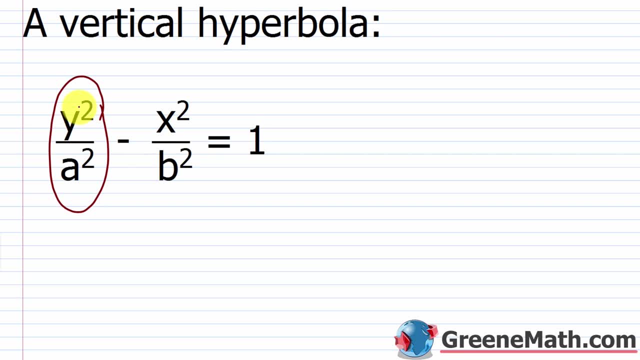 now. So it's a vertical hyperbola. Y is on the vertical axis, So we have y squared over a squared minus. x squared over b squared equals one. And again, when you think about the vertical ellipse, what was our formula there? It was x squared over b squared plus y squared over a. 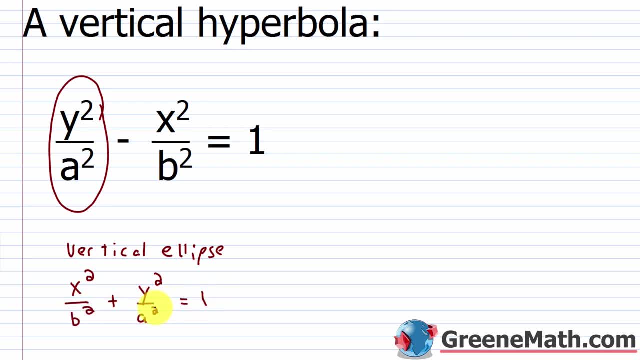 squared equals one. Now I could change the order of this around and put y squared over a squared first, because there's addition here. But I just want you to notice that the difference again is the plus sign here became a minus sign here. That's how you can tell if you have a hyperbola. 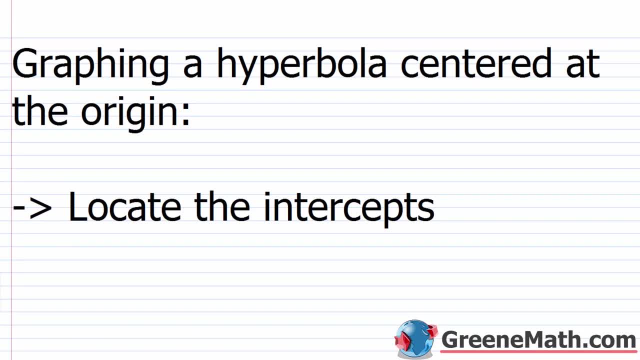 Now for today, we're just going to look at graphing a hyperbola that's centered at the origin. The first thing you need to do is locate the intercepts. If you have a horizontal hyperbola, you will have x-intercepts and no y-intercepts. 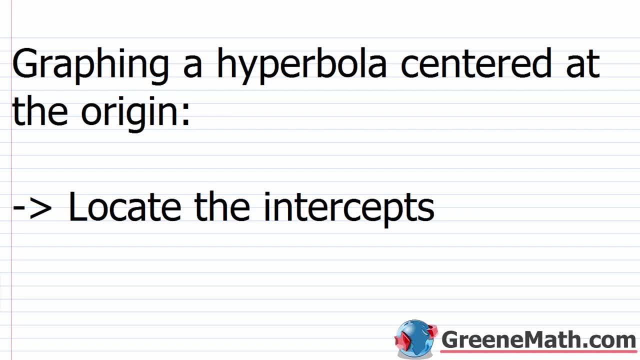 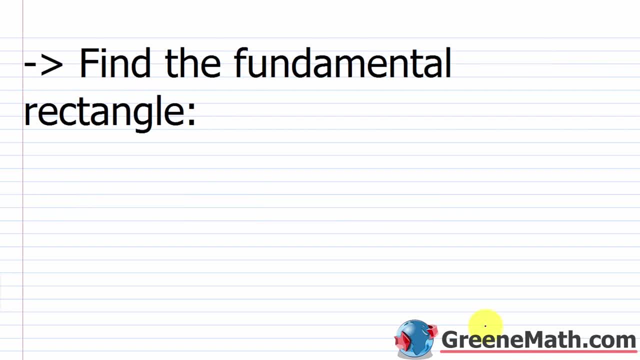 If you have a vertical hyperbola, you will have y-intercepts and no x-intercepts, And when we get to a problem, I'll show you why that's the case. The next thing you're going to do is find this fundamental rectangle, The points for this. I'll show you how to get those. You'll sketch the. 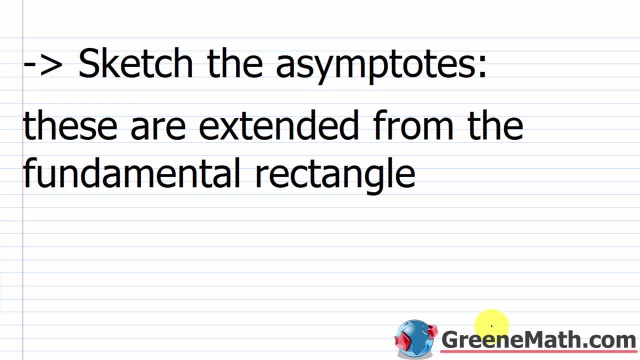 asymptotes. These are going to be lines that are extended from the fundamental rectangle, or you can actually get the equation for them from the hyperbola. You can graph them that way. Then, lastly, we will sketch the graph, So each branch of your hyperbola is going to have a horizontal 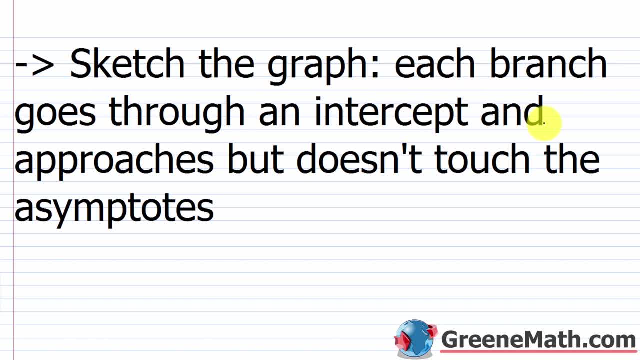 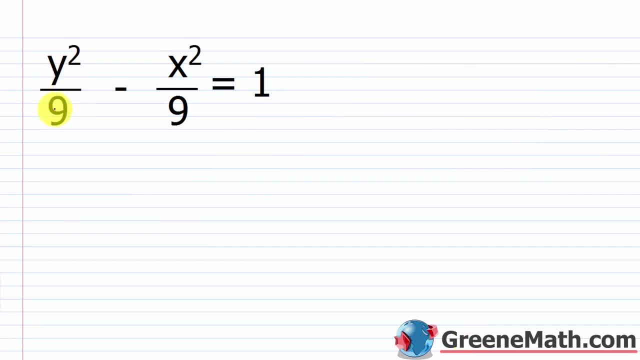 hyperbola that goes through an intercept and approaches but doesn't touch the asymptotes. So let's take a look at the first example. We have y squared over 9 minus x squared over 9 equals 1.. So in this case this term right here is larger, So it involves the y variable. 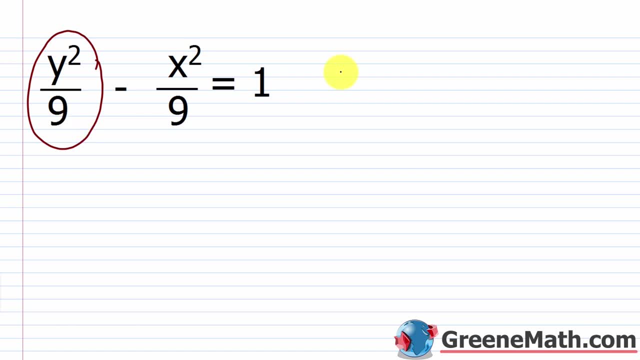 so I know I have a vertical hyperbola, So I know this guy is vertical. So what I told you is that if you have a vertical hyperbola, you will have y-intercepts and no x-intercepts. Why is that the case? We know how to find our x-intercepts and y-intercepts. If I want the y-intercept, 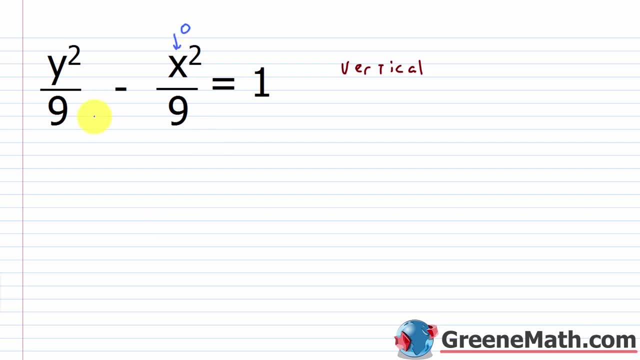 I plug in a 0 for x and I solve for y. We know that this would just go away. We know from our last lesson that the shortcut is: I can just take the positive and negative square root of that denominator there, Plus or minus. the square root of 9 is plus or minus 3.. So my y-intercepts. 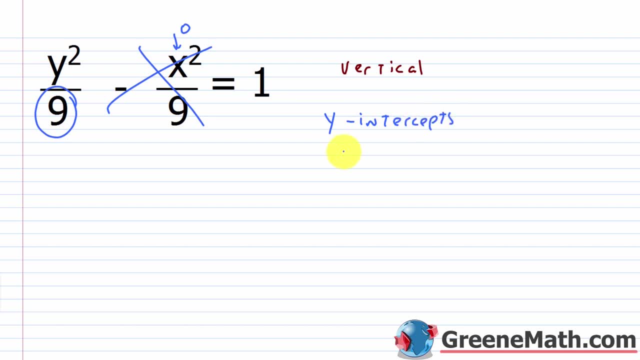 my y-intercepts would occur at 0,3 and 0 comma negative 3.. And you might say: where did that come from? Again, if I plug in a 0 here, that term's gone. So you would have y squared over, 9 is equal to 1.. To get y by itself, I would: 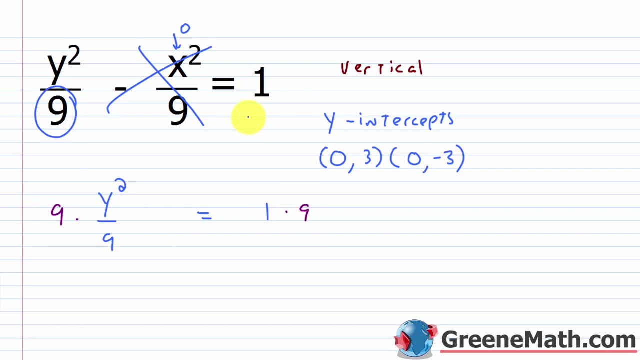 multiply both sides of the equation by 9.. Because in standard form this guy always is equal to 1. whatever the denominator was here, it always ends up on that side of the equation. So I end up with y squared is equal to whatever that denominator was. Now the end result to get y by itself is to: 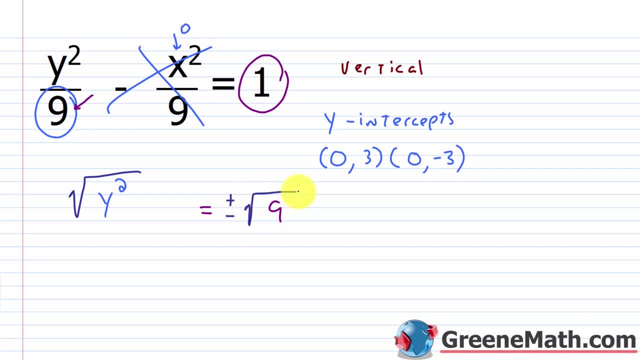 take the square root and over here I have to go plus or minus the square root of that guy. So the shortcut is always to look at the denominator and say plus or minus the square root of that. That will give me the y values for the y intercepts, And again you could do the same. 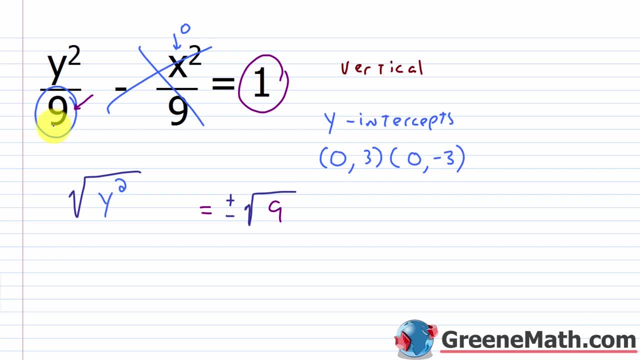 thing. if you're working with x intercepts, the concept is the same. So this gives me y is equal to plus or minus 3.. Of course, we already know that 0 comma 3 and 0 comma negative 3 are the y intercepts. Now you 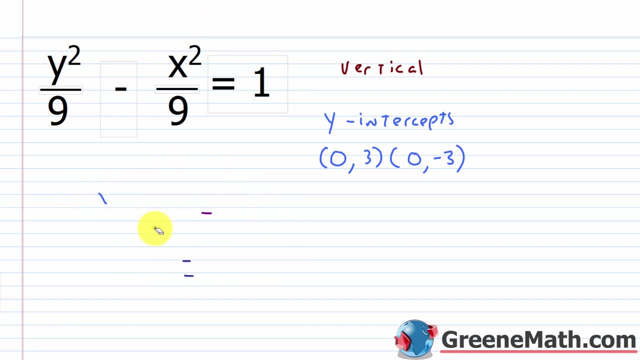 might say: why don't we have x intercepts? Why does that occur? Well, because of this minus sign here you're going to run into some problems. If I plugged in a 0 here and this term was gone, you'd have negative x squared over 9 is equal to 1.. Multiply both sides of the equation by 9. you'd 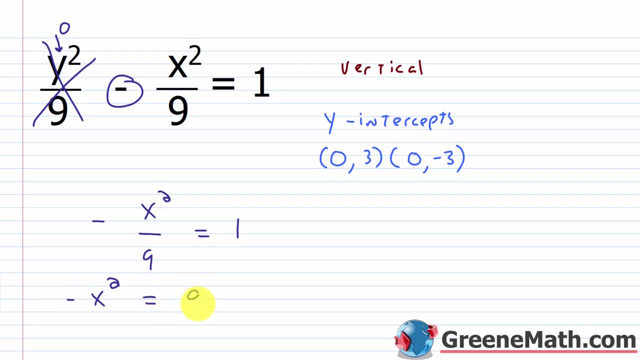 have negative x squared is equal to 1.. So you'd have: negative x squared over 9 is equal to 1.. Now let's say I divide both sides of the equation by negative 1 to get rid of that negative. So let's: 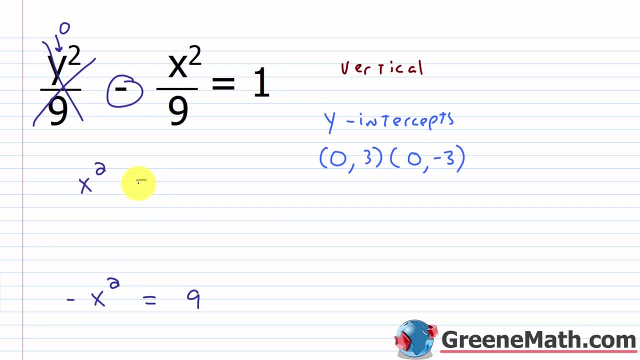 say, we have x squared now is equal to negative 9.. Is there a real solution that I can get there? No, there's not, Because if I take the square root of this side and I do plus or minus the square root of this side, the solution there is a complex solution, Although we can do it when we think. 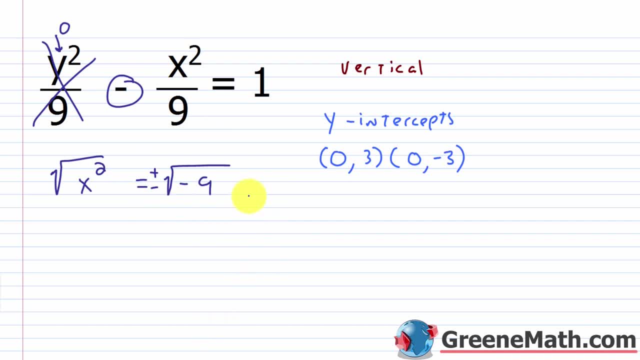 about just involving real numbers. we're not going to have a solution. So we're going to have a solution. So that's why we won't have any x intercepts here. So let's erase this. and a similar thing will happen when you have a horizontal hyperbola. Now we have our y intercepts. The next. 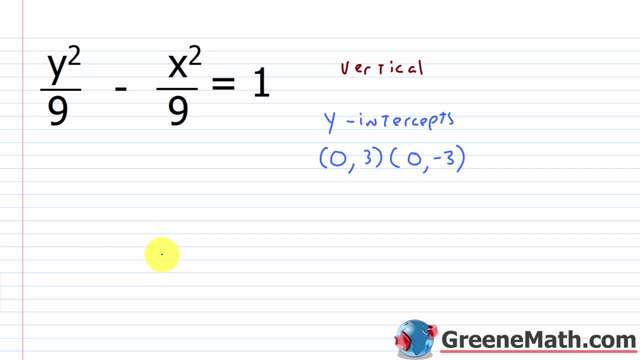 thing I told you you want to do is find this fundamental rectangle. So you'll see a formula for this in your book. The reason I don't teach this with the formula is because things are switching back and forth all the time. The a is different, the b is different. it's all over the. 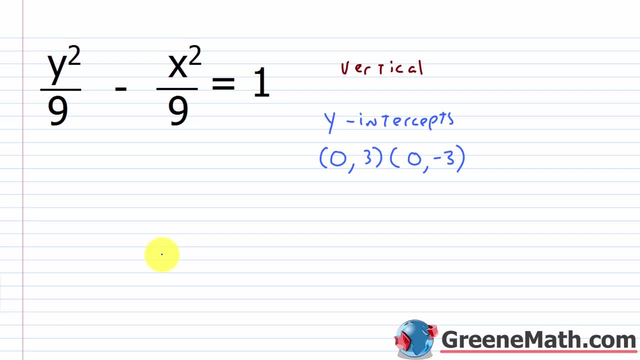 place and students have a hard time remembering, So I'm going to show you how to do this. So let's start by remembering, If you just remember, that the first point you want to get is x comma y. Where does x come from? Where does y come from? For x, you take the principal square root of that number. 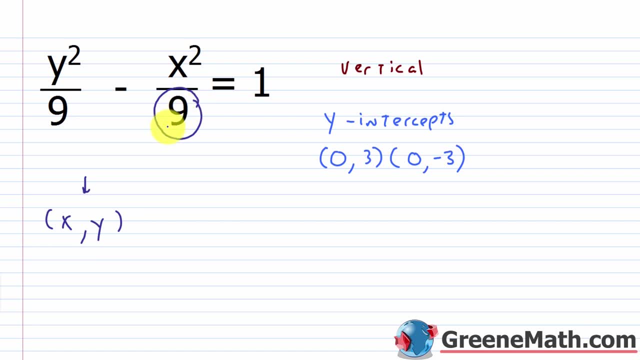 right there, Whatever's under x squared. So the principal square root of 9 is 3.. So it's 3.. Now for y. you take the principal square root of whatever is underneath the y squared variable. That's 3 also. Then you're going to do a variation of this, So there's four points total to make this. 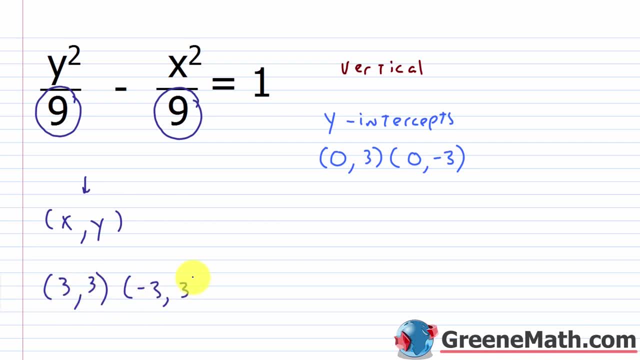 rectangle. So now I'll make this guy negative and this guy will stay positive, Then I'll make this guy positive and this guy negative, and then I'll make them both negative. Getting the fundamental rectangle is very, very easy if you just follow that formula there. 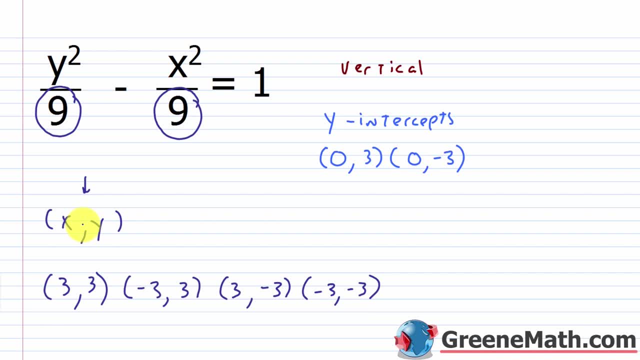 Again. just think about x and y in that format Now to get the asymptotes. they extend from the x to the y. So if you just follow that formula there, you're going to get the diagonal of this rectangle. So that's the easiest way to do it. If you want the formula for the 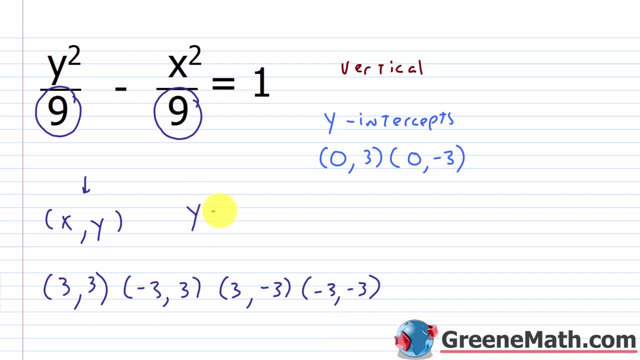 asymptotes. all you'd have to do is say y is equal to plus or minus. You'll have a slope here. then times x. Now where do I get this guy right here? Again, I want you to think about slope as rise over run. So there's going to be a vertical value that you move and a horizontal value that you move. 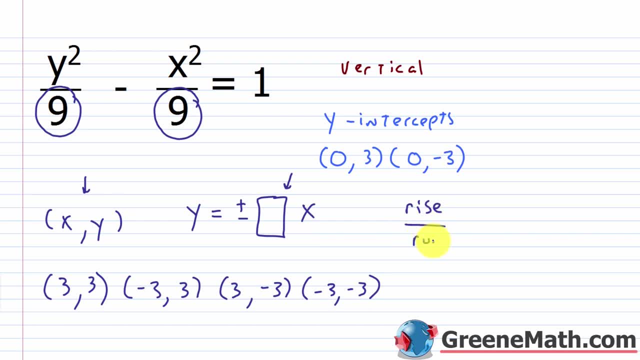 Again. think about rise over run. So where do I get the rise from? Again, you take the principal square root of this guy right here, whatever is underneath y squared, So that's going to be 3.. Where do I get the run? You go underneath. 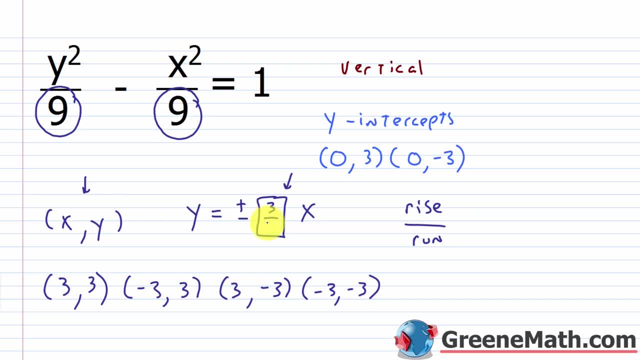 the x squared variable. take the principal square root of that, That's going to be 3.. In this particular case, we have the same denominator in each case, So it's really really easy, right? We know that it would be 3 over 3 or just 1.. So this is 1x and you're going to have two scenarios. So 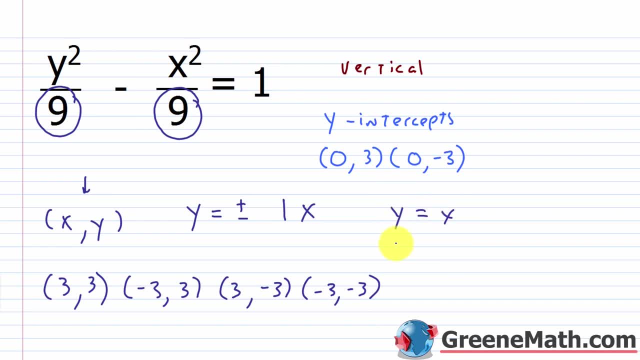 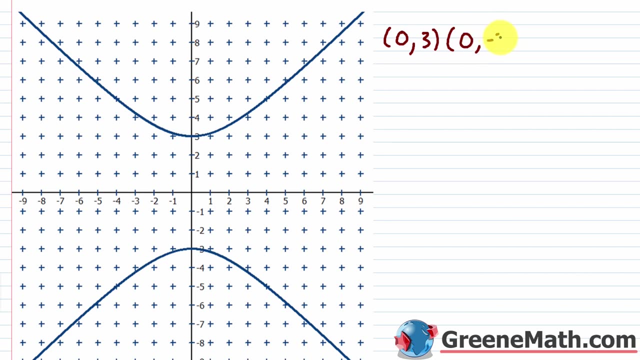 one line would be: y is equal to x. The other line would be: y is equal to negative x. So let's take all of this information to the coordinate plane and I'll show you how to sketch the graph. So let's start out with the y intercepts. They occurred at 0 comma 3 and also 0 comma negative 3.. So 0 comma. 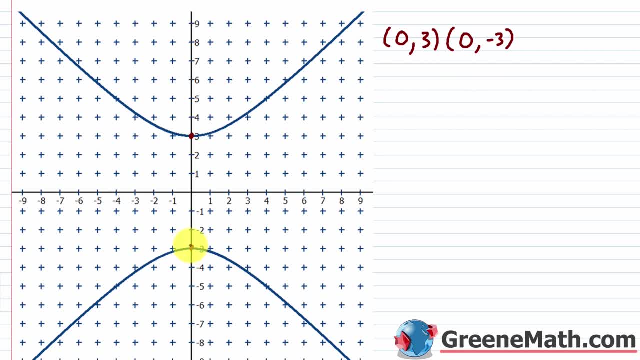 3 is right here, 0 comma negative 3 is right here. Then let's think about that rectangle. So we know, they were at 3 comma negative 3. Then we had negative 3 comma positive 3. And then we had 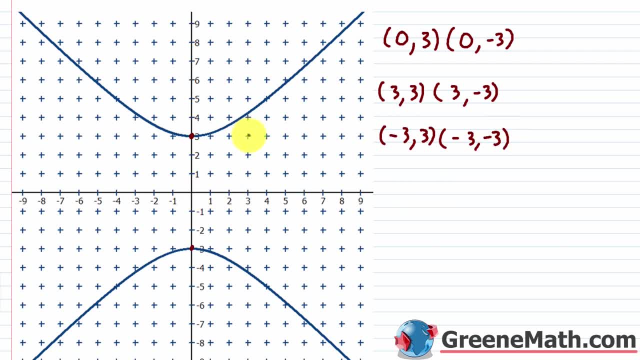 negative 3 comma negative 3.. So 3 comma 3 is right here, 3 comma negative 3 is right here, Negative 3 comma 3 is right here, And then negative 3 comma negative 3 is right here. So now we would connect. 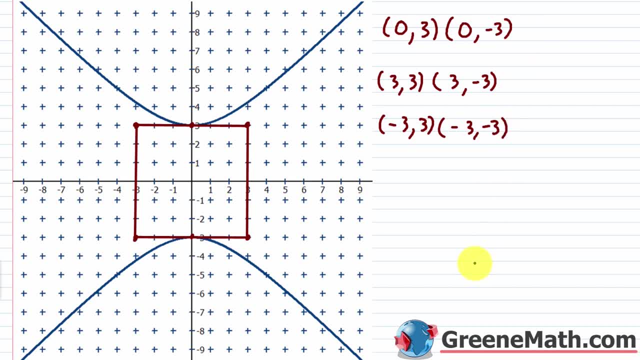 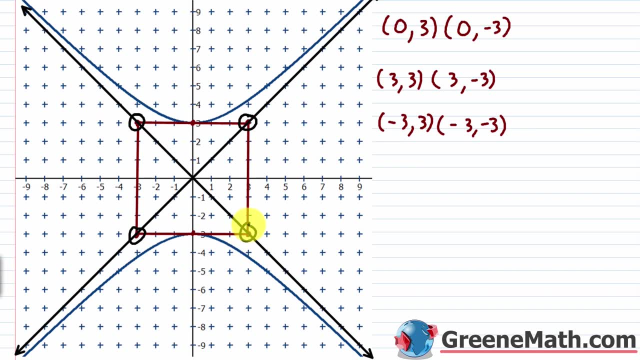 them, And in the 3 comma rectangle drawing you can extend from the diagonals your asymptotes. So you can either again extend these from the diagonals there Or you could just find the asymptotes on your own. again, We found that it was y equals plus, or 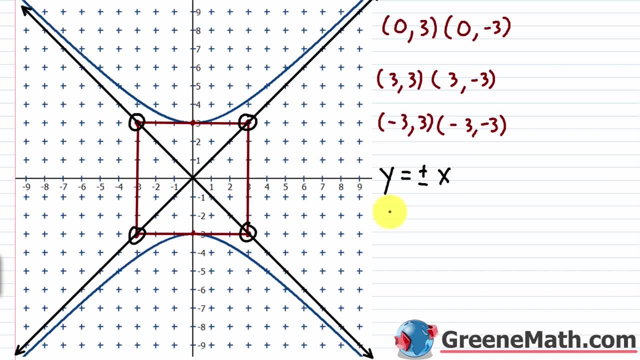 minus 3 over 3, which is 1 times x. So this is y equals x or y equals negative x. So if you did y equals x, that would give you this guy right here, this line, right here, this is y equals x. So if I start at the origin, I go up one. 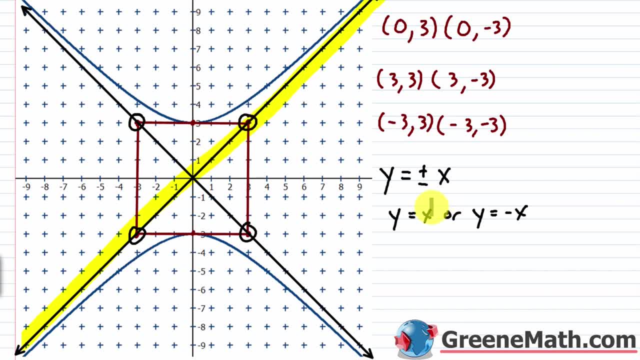 I go to the right one up, one to the right one, you know, so on and so forth. Y equals negative x. that's going to be this guy right here, And that's y equals negative x. Now, once you have all that drawn, you would think about the. 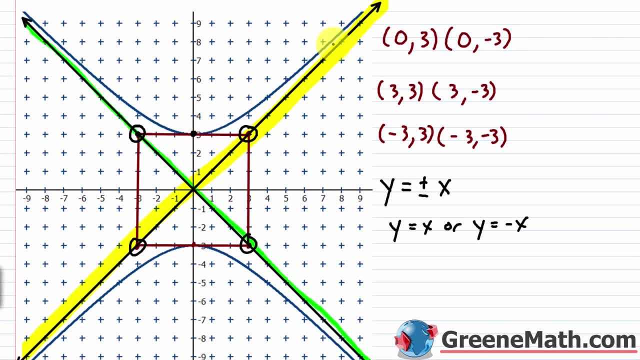 actual hyperbola. So I've had the computer draw this for us, just so it's accurate. but I'm going to trace over it. And again, when you draw this, each branch is going to go through an intercept and approach but not touch the asymptote. So let's kind of start here and we'll come down. 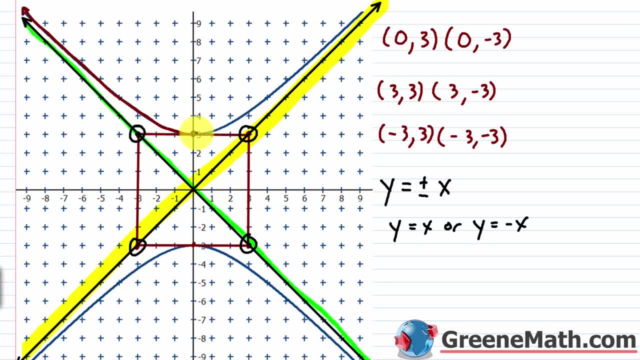 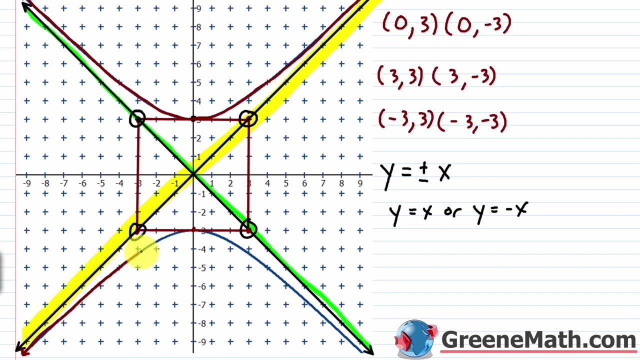 And again we'll go through this intercept here and we will come back up And again we approach the asymptote but we don't touch it. Let's do the same thing down here. Okay, so we'll take this 3x. 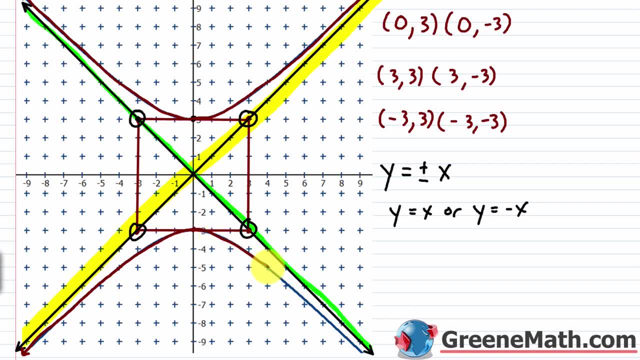 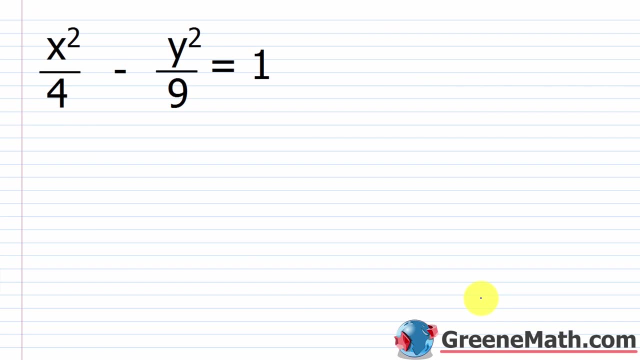 we approach the asymptote but we do not touch it. And again, not perfect, but you're giving a general idea of what this guy looks like. Let's take a look at another one. So we have x squared over 4 minus y squared over 9, and this equals 1.. So in this case, this guy right here is the. 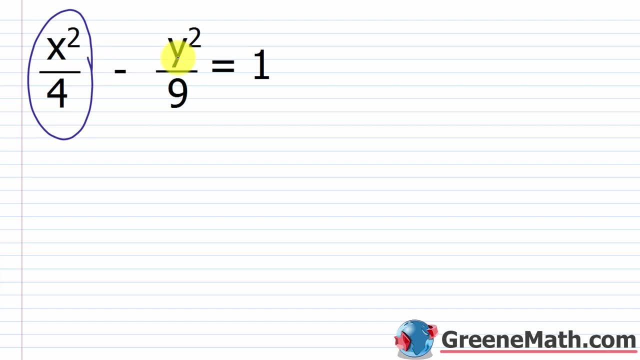 dominant one. We know this is larger because this minus the y, squared over 9, is equal to 1.. So again, this will tell me that if the x variable is involved in the larger term or the term, that's positive, however you want to think about that, it's a horizontal hyperbola With a horizontal 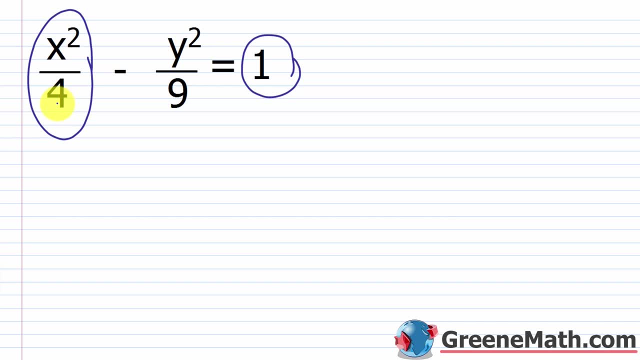 hyperbola, I'll have x intercepts and no y intercepts. So how do I get my x intercepts? The shortcut is to take that guy right there and take the principal and negative square root of that. So plus or minus the square root of 4 is plus or minus 2.. 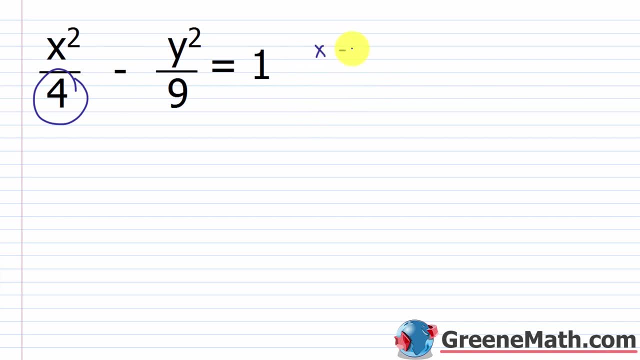 So my x-intercepts, my x-intercepts occur at 2, 0 and negative 2, 0.. All right, let's talk about the fundamental rectangle. So our rectangle Again, how do we get these endpoints? I'm just going to say x, y. 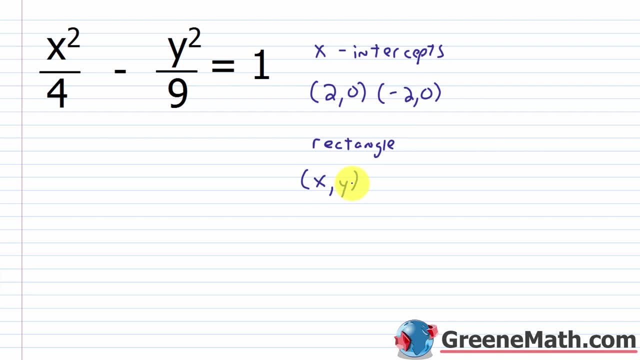 With the formulas you get in your textbooks. again, they go back and forth based on what's a, what's b. It's kind of all over the place and it takes a lot to really memorize that stuff. If you just think about the fact that you're going to have an x value and a y value, it's 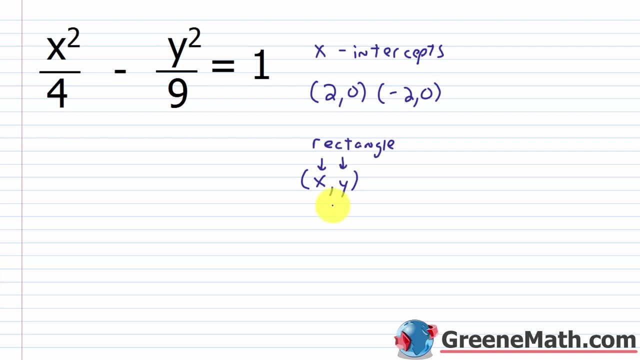 very easy to get this. So, for the rectangle, think about the first point that you would have. So it's x, y. Where does x come from? Take the square root of whatever's under x squared. The square root of 4 is 2.. 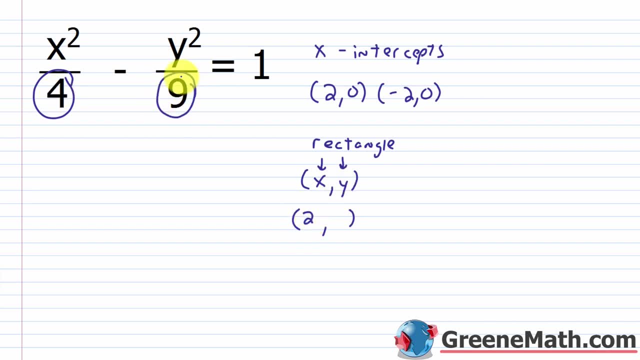 Where does y come from? Take the square root of whatever's under y. squared Square root of 9 is 3.. So it's 2,, 3, and then I get variations of that, So I end up with negative 2.. 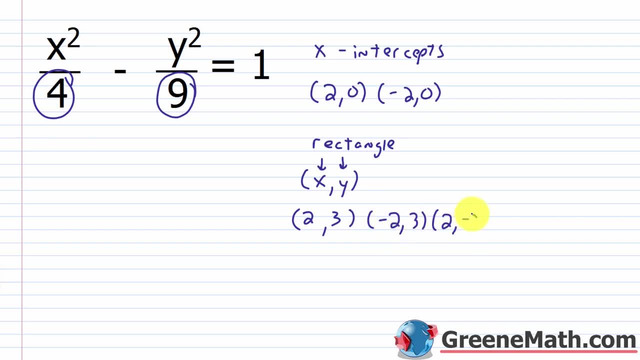 I end up with 2, 3.. I end up with 2, negative 3, and I end up with negative 2, negative 3.. Very easy once you think about it. that way, You never have to remember any kind of crazy formulas. 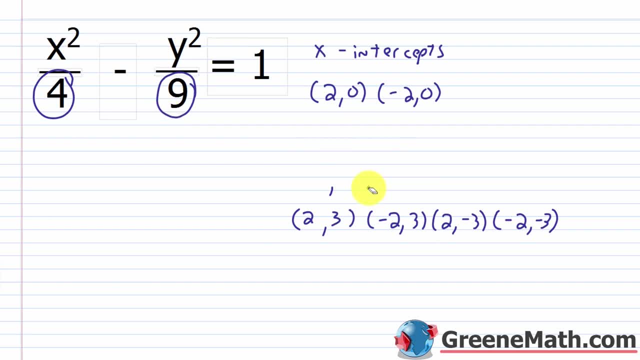 None of that. You get your rectangle right away. And some people don't even want the rectangle, They just want the asymptotes. You can do that too. The asymptotes are easy to find also. So y equals: you have your slope times, x, right? 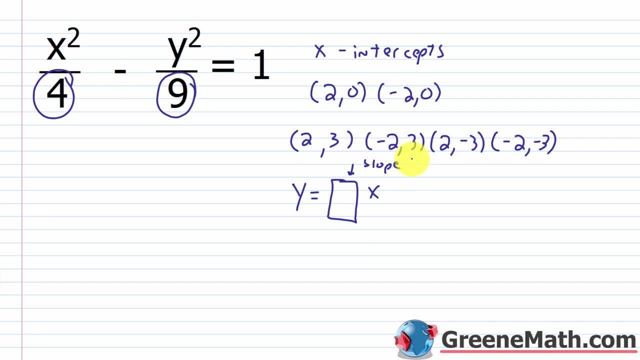 Your slope Again. what is slope? It's rise over run. Well, where do I get the rise from? Again, rise is vertical. We're thinking about the y variable. Again, take the principal square root of 9.. That's 3.. 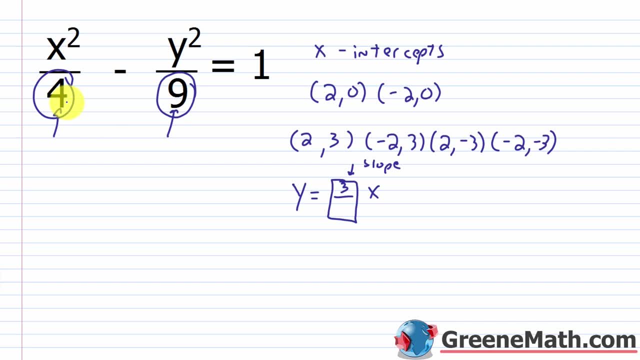 Then for the run, take the principal square root of 4.. That's 2.. So you would have y equals plus or minus 3 halves x, Plus or minus 3 halves x. okay, That would be your two equations for the asymptotes. 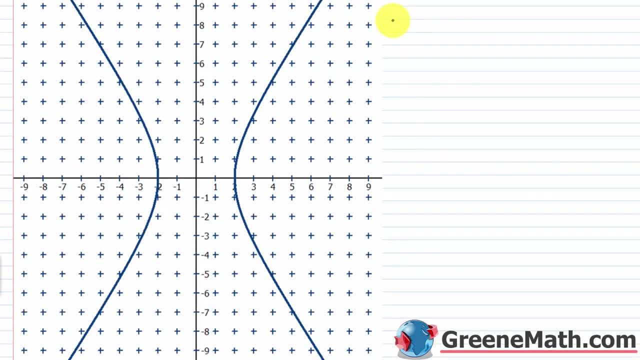 So let's take this information to the coordinate plane Again, we saw that the x intercepts are going to occur at 2, 0 and then negative 2, 0. So 2, 0 is here. Negative 2, 0 is here. 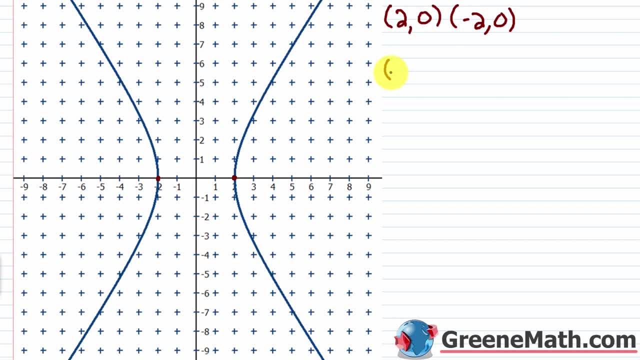 We found that the fundamental rectangle endpoints were what We had: 2, 3.. We had negative 2, 3.. We had 2, negative 3.. And then we had 2, 3.. And then we had 2, 3.. 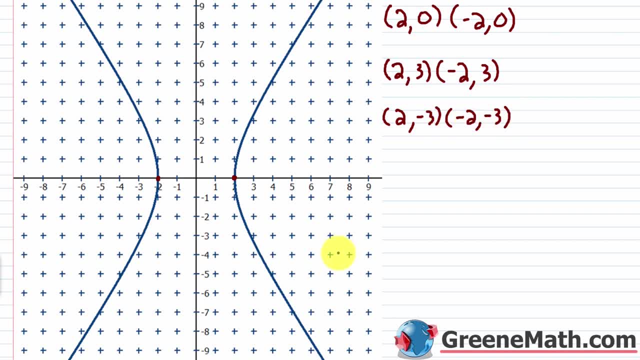 And then we had negative 2, negative 3.. So 2, 3 is right here, Negative 2, 3 is right here, 2, negative 3 is right here And negative 2, negative 3 is right here. 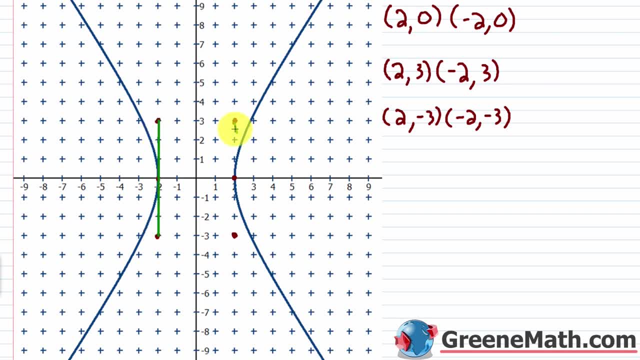 Let's go ahead and make this rectangle, Okay. And again, once this is drawn, I can extend my asymptotes from the diagonals. So from here and here I could make a line going through that. And then from here and here I can make a line going through that. 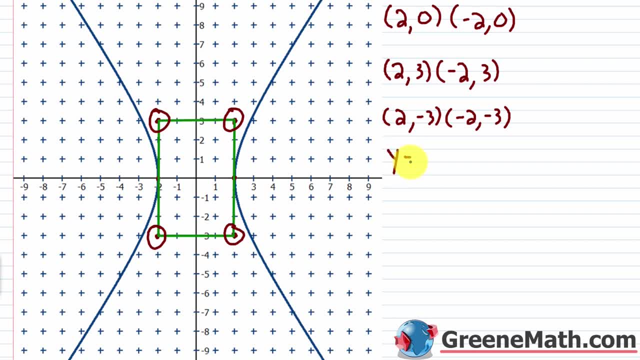 Or again, I could just find the equation. We found that it was y equals plus or minus 3 halves x. So y equals 3 halves x and y equals negative 3 halves x. So if I started at the origin, if I went up 3 units- so 1,, 2,, 3, and I went to the right 2,. 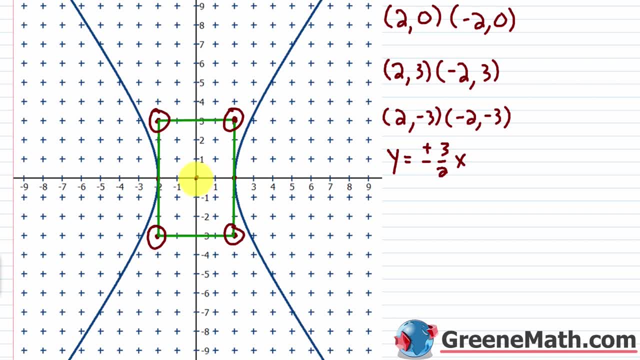 that would put me at that point there, If I went from the origin down 3 units- 1,, 2,, 3, and to the left 2, that puts me right there. So you can see that would be the line. 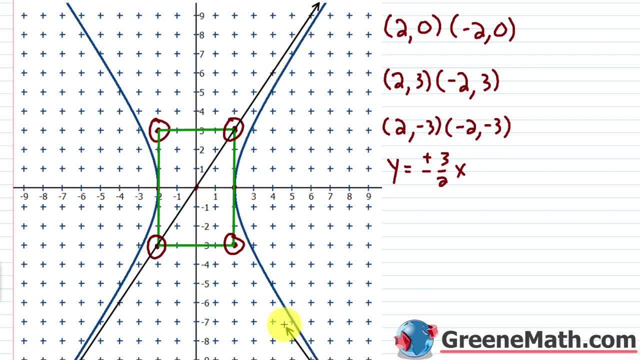 So let's go ahead and sketch that guy. So let's graph the hyperbola now. So I would again approach the asymptotes, but I wouldn't touch them. And this guy is going to go through the intercept And coming back around. I'm approaching the asymptote, but I'm not going to touch it. 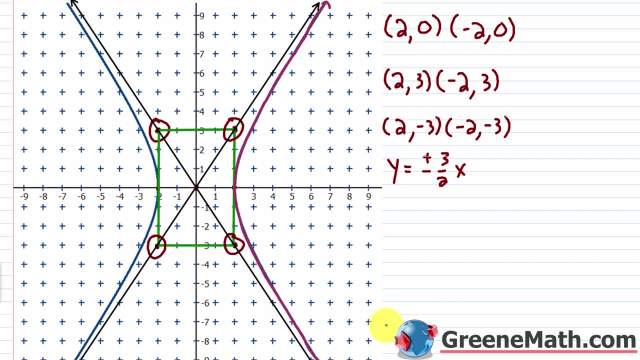 But again pretty hard to do. I could do this freehand and be accurate, but that's why I pre-drew everything just to make it a little bit better. Again through the intercept and then approaching the asymptote and not touch it. 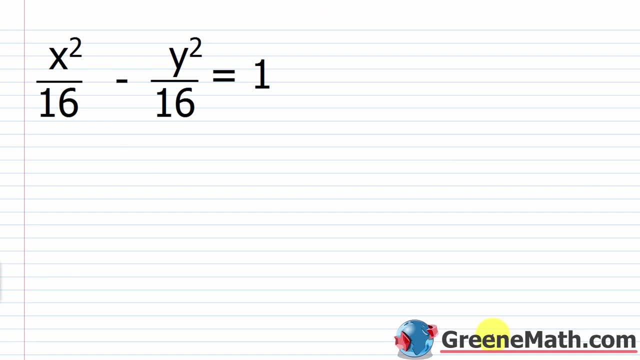 Let's take a look at one more. So we have x squared over 16 minus y squared over 16 equals 1.. Again, this guy right here. you think about this as being the positive one, or the larger one the more difficult. 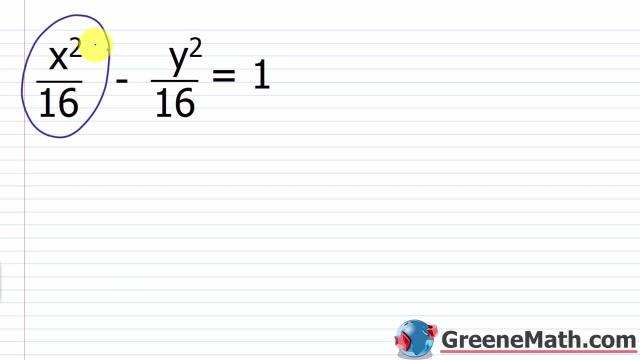 In the end, x squared over 16 minus y squared over 16 is 1.. So this guy has to be bigger. So this is going to be a horizontal hyperbola. So again we'll have x intercepts and no y intercepts. 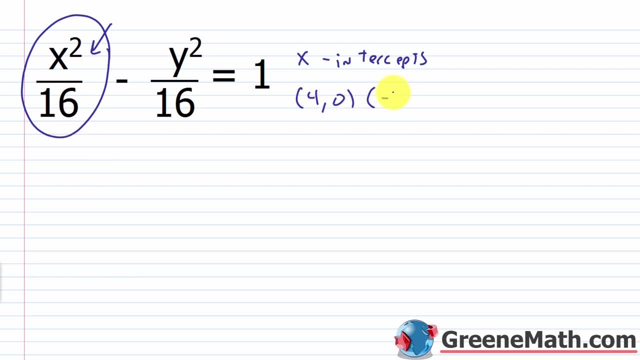 So those would occur at 4 comma 0 and negative 4 comma 0.. I got that by taking the principal and negative square root of 16, right Plus or minus. the square root of 16 is plus or minus 4.. 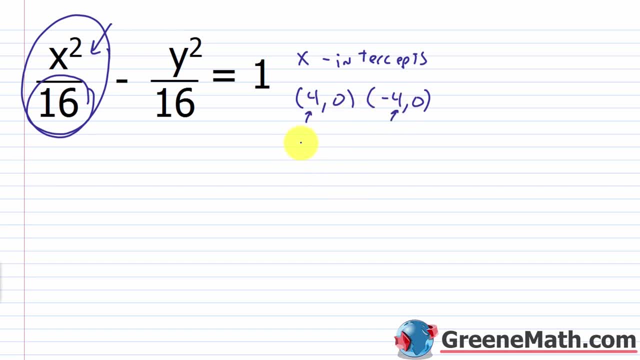 That's how I get the x, That's how I get the values there and there. Getting the fundamental rectangle here is very easy because I have the same denominator in each case. So I know it would be 4 comma 4 to kind of get things started. 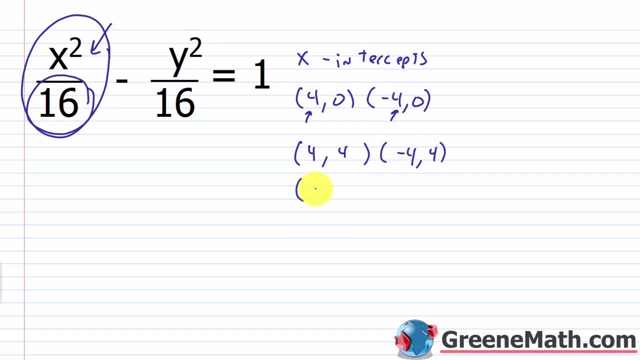 And then I would do negative 4 comma 4.. I would do 4 comma negative 4.. And then I would do negative 4 comma, negative 4.. And again, this is all you really need. You can extend your asymptotes from the diagonals of the rectangle. 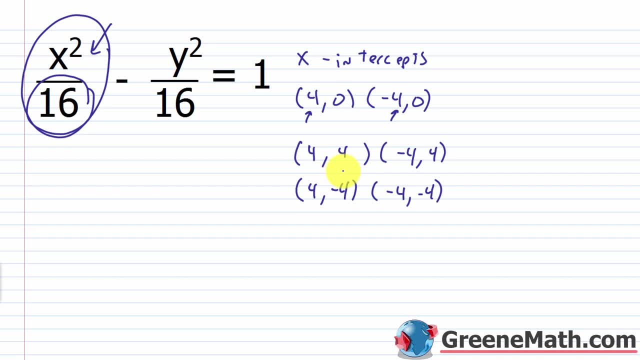 or you can just figure out what the asymptotes are. In this case, again, you have 4 and 4. If I think about the square root of 16 and the square root of 16.. So the asymptotes would just be: y equals plus or minus. 4 over 4 is 1.. 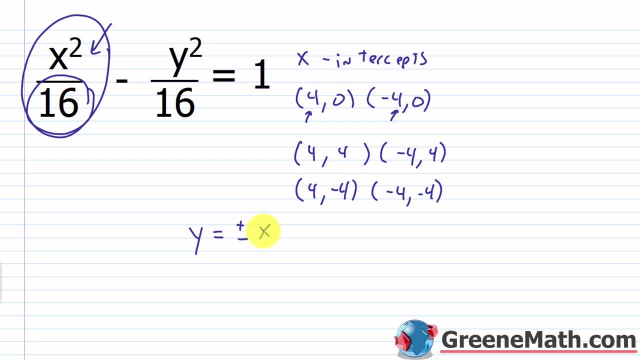 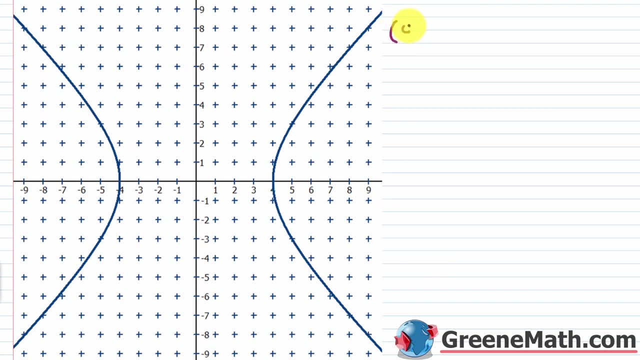 So y equals plus or minus x. All right, So let's take this information and let's graph this guy real quick. So again, the x intercepts occurred at 4 comma 0 and you had negative 4 comma 0.. So 4 comma 0 is here. 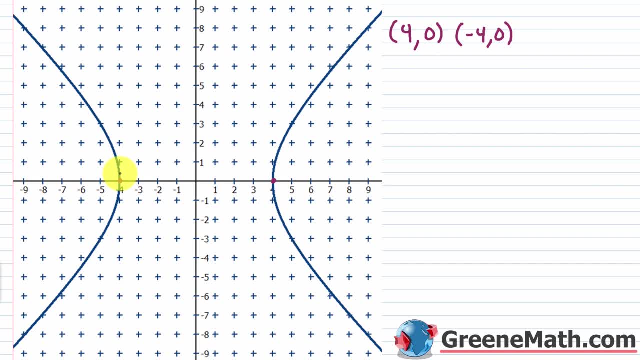 Negative 4 comma 0 is here. Then for the rectangle, again we had the point It's 4 comma 4,, you had negative 4 comma 4, you had 4 comma negative 4, and you had negative. 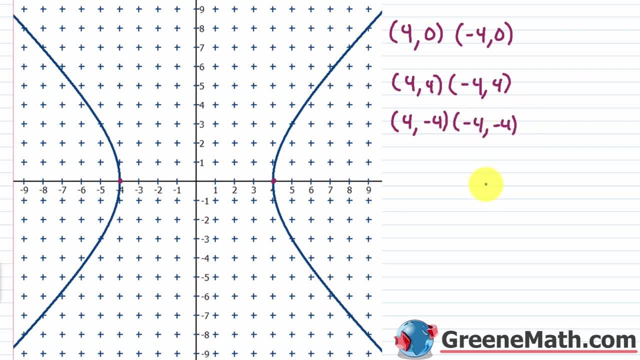 4 comma negative 4.. So for 4 comma 4, that's here. For negative 4 comma 4, that's here. For 4 comma negative 4, that's here. And then for negative 4 comma, negative 4, that's here. 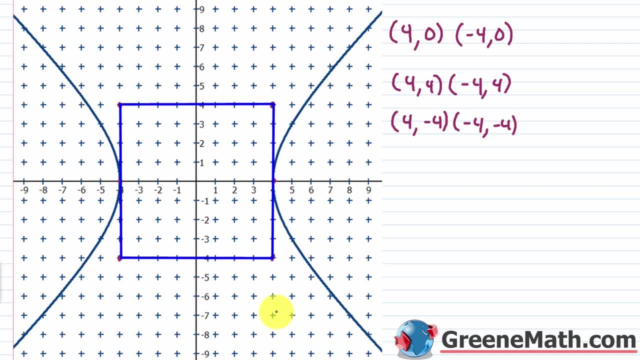 Okay, So the rectangle is drawn Again. if I want to, I can just extend the diagonals there and create my asymptotes. Or again, I know it's y equals x or y equals negative x. So, starting here, I would go up 1 and to the right 1, up 1 and to the right 1, you know. 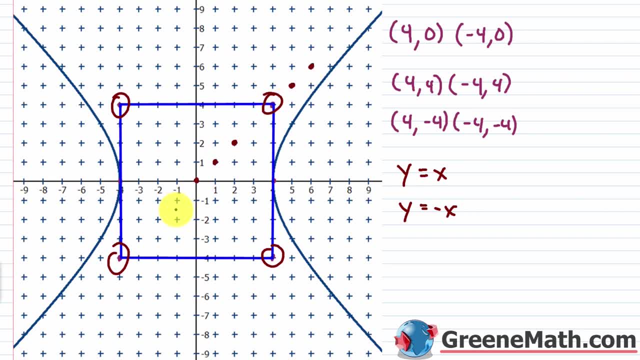 so on and so forth until I got to that point, this point, this point We're going down. It's the same thing For the other guy. if it's y equals negative x, I would go down 1 and to the right, 1,. 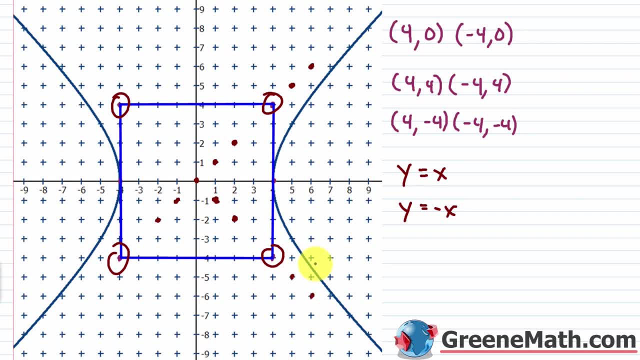 down 1 and to the right 1, you know so on and so forth. Okay, I'd have points down here. I could also make points going up here, Okay. So let's draw the asymptotes. So I have my asymptotes drawn. 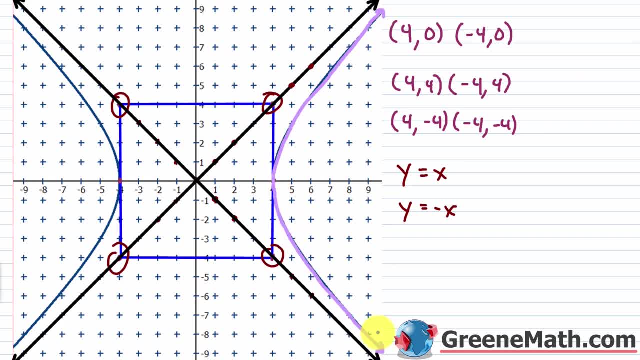 Again, it goes through the intercept. Again, it goes through the intercept. Okay, Again, not perfect, but you get the general idea of what the shape is, and that's all we're looking for when you're asked to do this freehand. 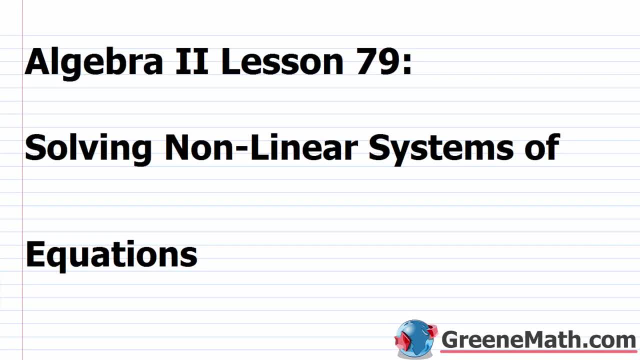 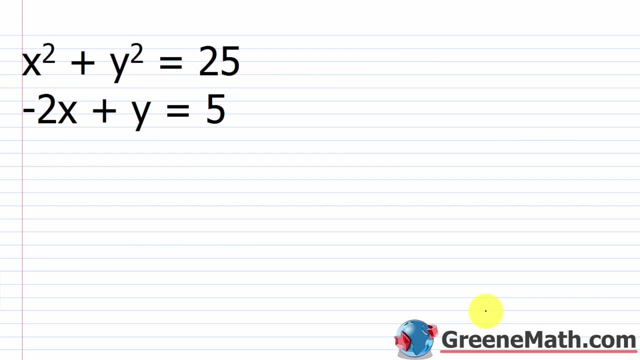 Hello and welcome to Algebra 2, Lesson 79. In this lesson we're going to learn about solving nonlinear systems of equations. So at this point in Algebra 2, you should be very comfortable with solving a system of linear equations in 2 variables or 3 variables using substitution. 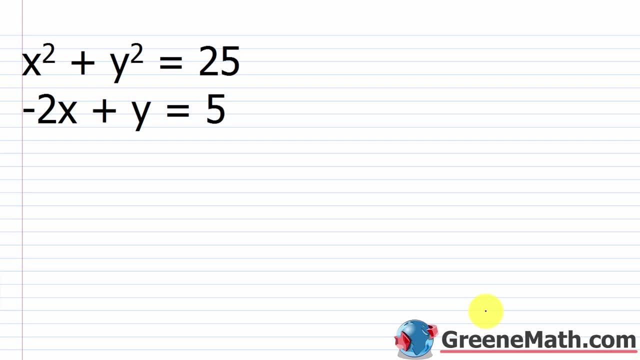 elimination, graphing or matrix methods. Here, what we're going to do is just introduce something new. The concept is very much the same, though. The only difference here is you just have to be very, very selective about what method you're going to use, based on the situation that you're in. 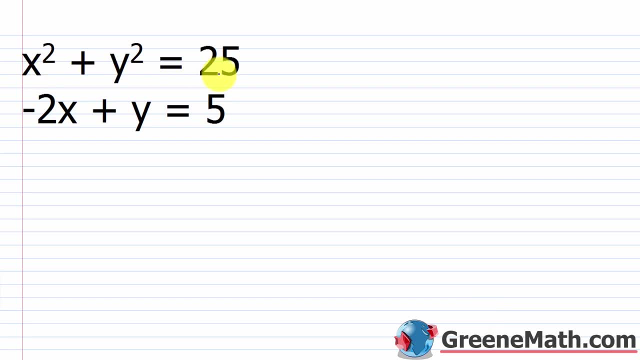 So the first thing that we're going to look at: we have a second degree equation here. We have x squared plus y squared equals 25.. We know this is the equation of a circle. Then we have a line, So we have a linear equation here as well. So the definition of a nonlinear system just has to have 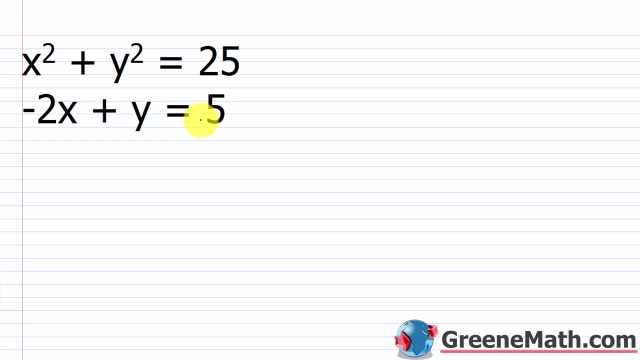 one nonlinear equation involved. So if we wanted to solve this type of scenario, we're going to turn to substitution And you can see with this linear equation what happens is I have a y here that has a coefficient of one, So very easily I can solve. 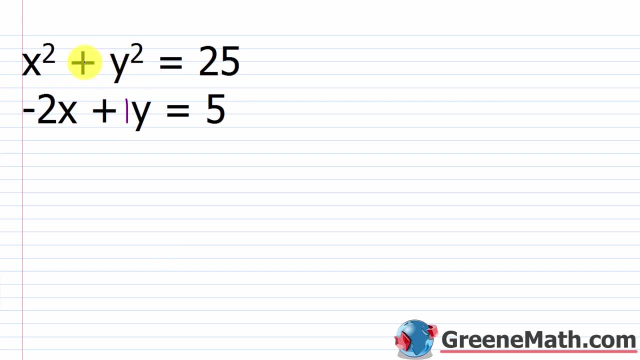 this guy for y and I can substitute into this kind of top equation. So the first thing I'm going to do is I'm going to label this equation up here as equation one, and this guy right here is equation two. So I'm going to solve equation two for y. So let's start with that. So I have. 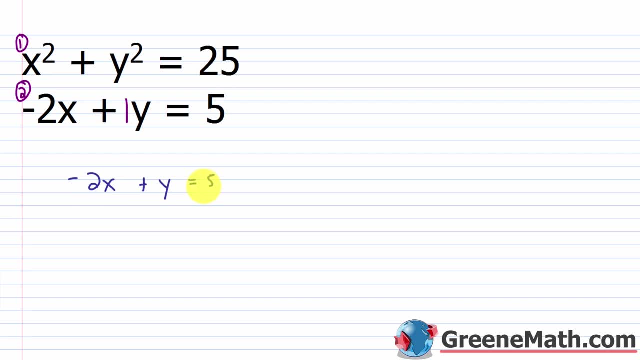 negative: 2x plus y squared. So I'm going to solve equation two for y. So let's start with that. y equals five. Very easy, I'm just going to add 2x to both sides of the equation And this is going to cancel. So what I'll have is y is equal to. we'll have 2x plus five. 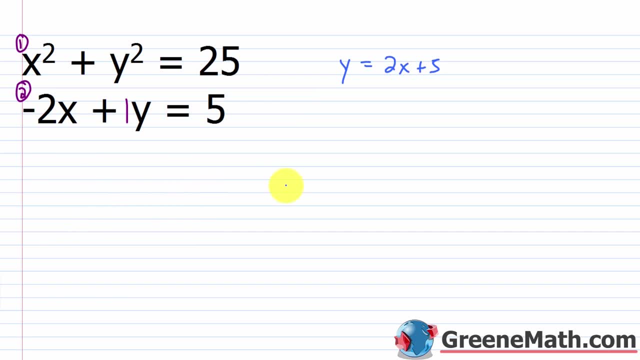 Let me erase this. Now. with substitution, we remember that we substitute in for the variable, So I'm going to substitute in for y and I'm going to substitute in here. right, I'm not going to substitute in from where I took it from, So I'm going to substitute in for y and I'm going to. 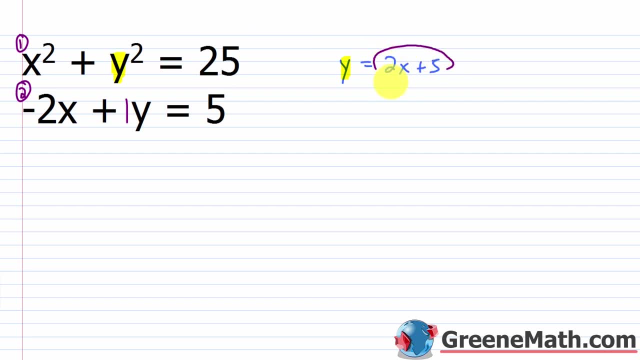 substitute in for y. So I'm going to take this 2x plus five and I'm going to plug that in right there for y. So that would give me x squared plus. I want this whole thing to be squared. I'm plugging in a 2x plus five there. So the quantity 2x plus five, the whole thing needs. 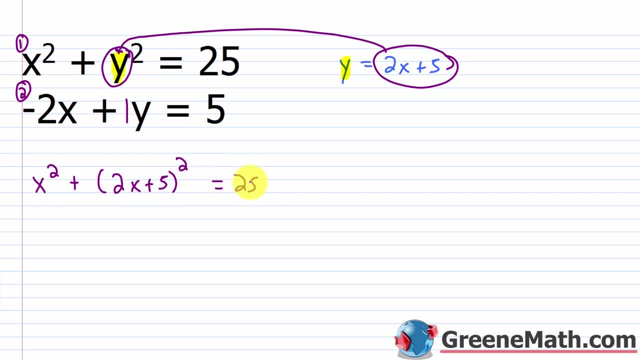 to be squared, Then this is equal to 25.. Now that we have that out of the way, once you've got that concept down, it's just pretty much some simplification from that point. So we have x squared plus. I'm going to square this guy. I can use my special products formula. I know that. 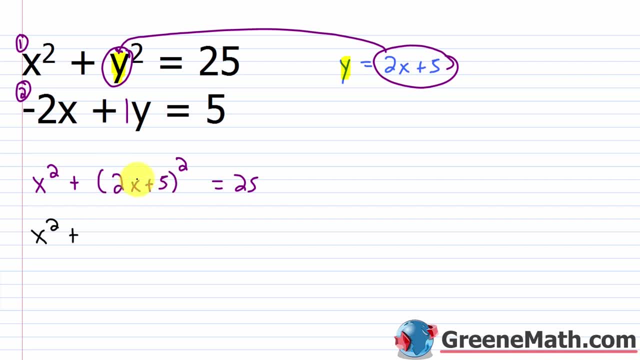 I would take this first guy, this 2x, that term, and I would square it: 2 squared is four, x squared is just x squared. Then, plus two times this guy, times this guy Two times 2x is 4x, 4x times five. 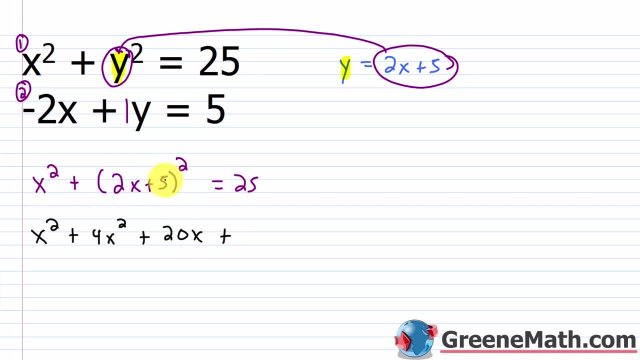 is 20x, Then, plus this last guy, five squared, which is 25.. And then this equals 25.. So the first thing we can do is subtract 25 away. So we're going to subtract 25 away from this guy. 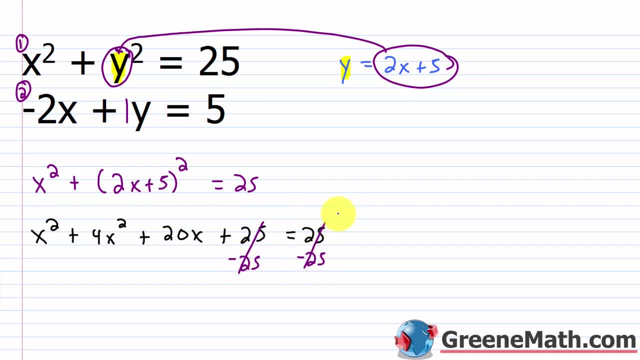 So that'll go away and that'll go away. I'll have a zero over here And what I'll have is x squared plus 4x squared, which is 5x squared, Then plus 20x, and this equals zero. So let me. 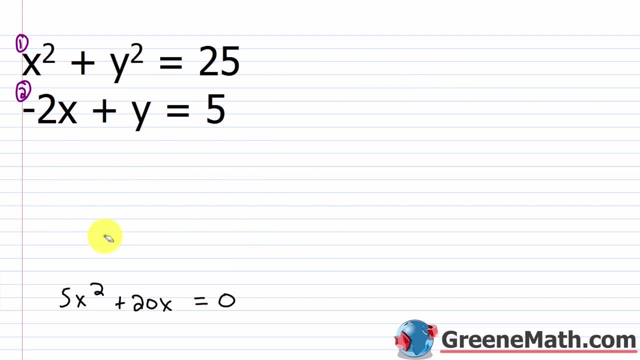 erase everything to this point. I don't need any of this. Now. how can I solve this for x? Well, we have a few different things we can do. We could use our quadratic formula, but kind of the quickest way to do this here is to 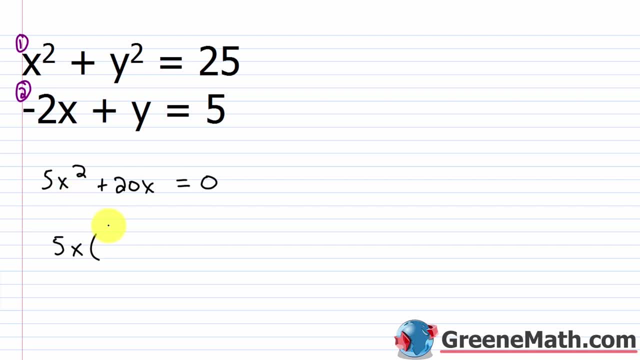 factor it. I could factor out a 5x and I could write this as x plus 4 inside the parentheses. I could say: this is equal to zero. So now I can use my zero factor property, or you could say the zero product property, And I could set each factor equal to zero. So I could say: 5x equals zero. 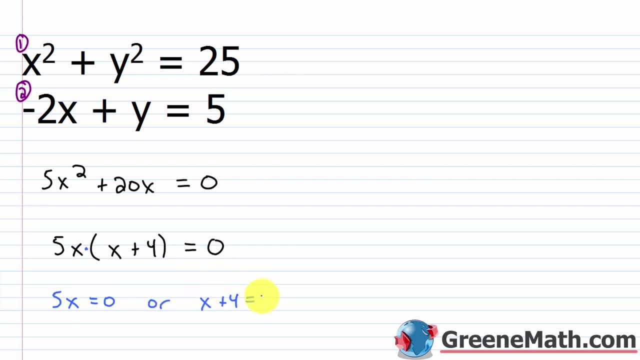 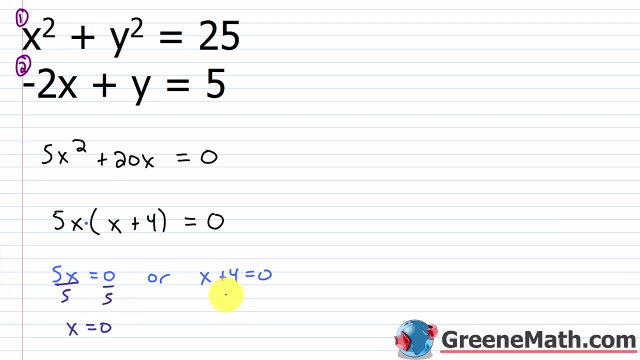 or the quantity x plus 4 equals zero. If I solve this, I divide both sides by five and I get x equals zero over here. If I solve this, I subtract four away from each side and I get x equals negative four over here. 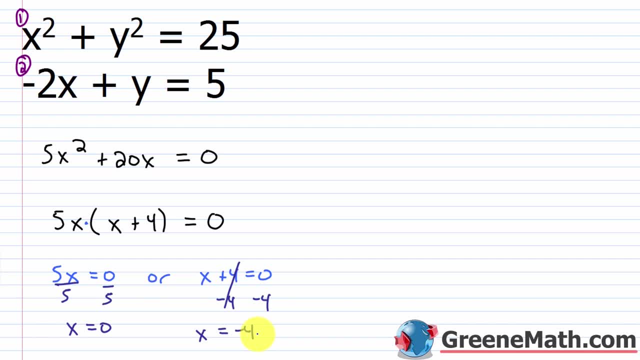 So I'm not done. I have found out two solutions for x, but I don't know the corresponding y values. So one x value would be x equals zero. The other x value would be x equals negative four. So let's erase this, All right. so if x equals zero, what is y? So I'm going to plug a zero in. 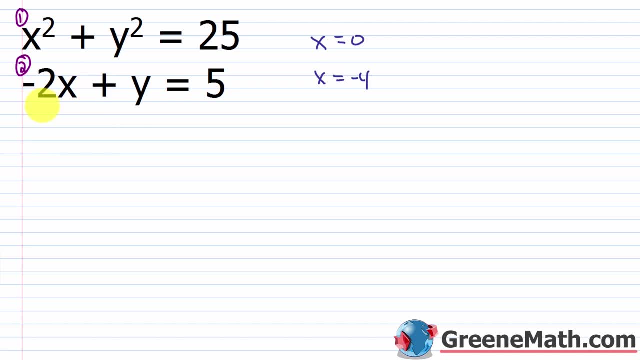 for x in one of these equations, Doesn't matter which one. I want to pick the linear equation because it's easier to work with. So I would say negative. two times zero plus y equals five, And so this is going to go away. 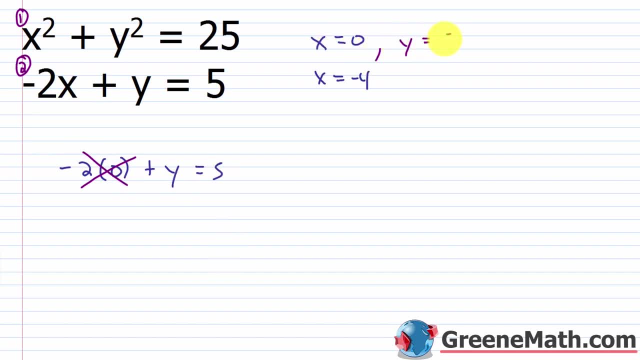 I'll have: y equals five. So if x is zero, y is five. Now the other scenario occurs when x equals negative four. So we'd have negative two times negative. four plus y equals five. Negative two times negative. four is positive eight. So eight plus y equals five. We will subtract eight away. 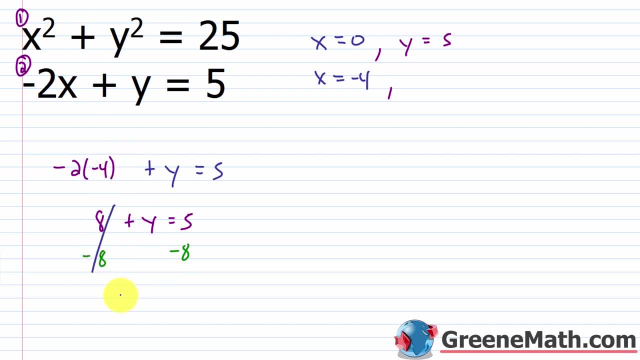 from each side of the equation Cancels, We'll have: y equals five minus eight is negative three. So if x is negative four, y is equal to negative three. Now, I'm not going to do this in every video, but I do want you to. 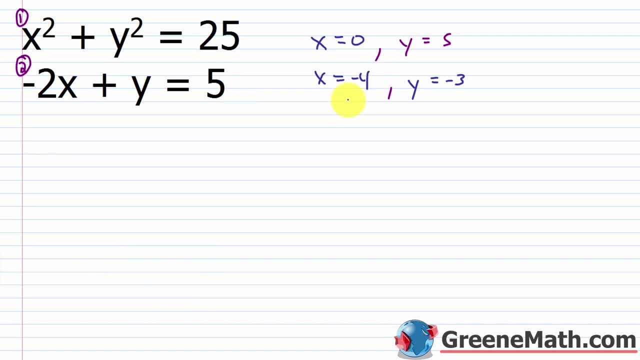 understand that you should check these solutions and make sure they work in each equation. So if x equals zero, y equals five, that's the ordered pair. zero comma five. Then if x equals negative four, y equals negative three, That's the ordered pair. 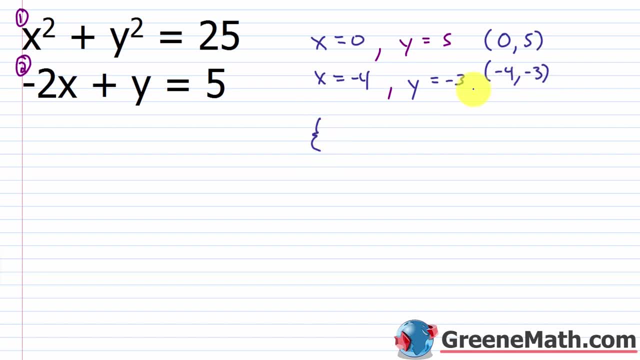 Negative four comma negative three. So in solution set notation put zero comma five and negative four comma negative three. All right, So let's check these guys real quick. So I'm going to check zero comma five in each one real fast. So zero squared plus five squared. 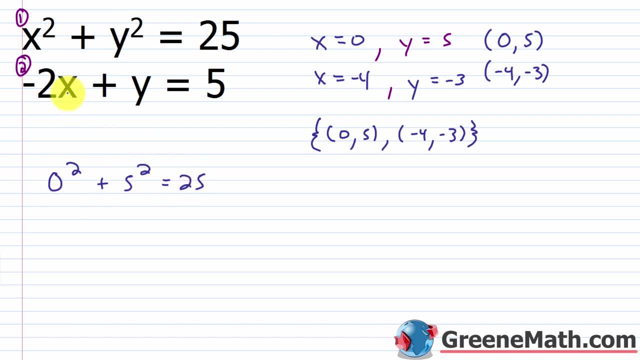 equals 25.. We know that works. Then what about here? If I had zero here and five here- we know that works as well- right, This would go away. You'd have five equals five, All right. So this guy is a solution. 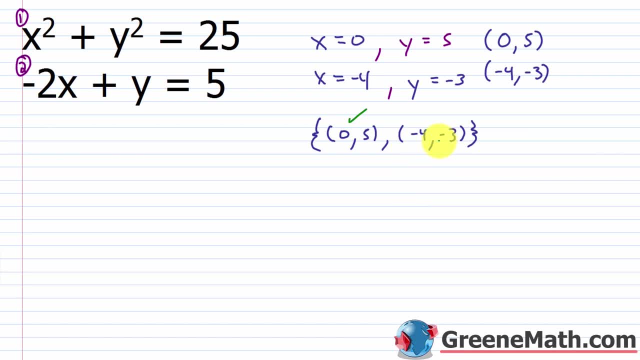 For both. this one checks out: What about negative four comma, negative three. So negative four squared plus negative three squared equals 25.. Negative four squared is 16.. Negative three squared is nine. 16 plus nine is 25.. So it does work there. All right, Let's check it in the last. 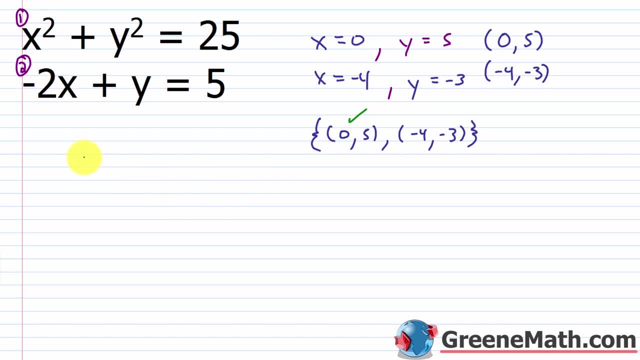 one, So negative, two times negative, four would give me eight, So I would have eight plus negative three equals five. We know that's true. All right, So let's check out in each one as well. All right, So I'm not going to check each one. 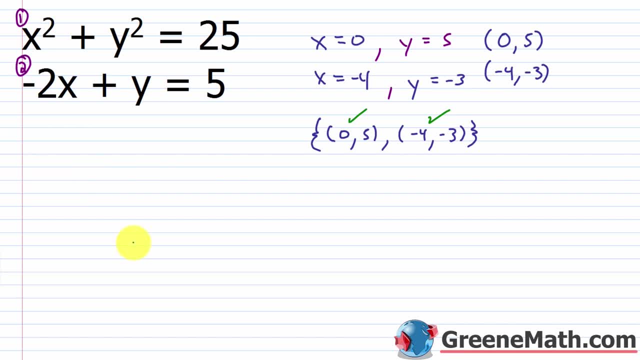 moving forward. I've already checked these. It's something you can do on your own for practice. I just really recommend you check things, especially when you're on a test and you're trying to get all the credit that you can. Now I want to show you something before we kind of move on. I've 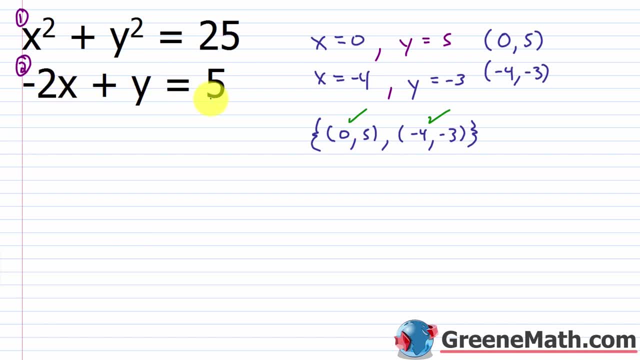 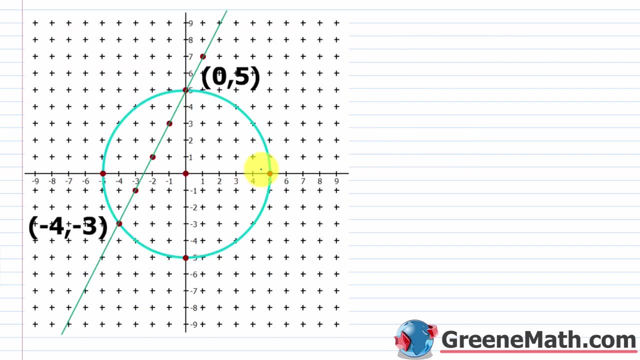 graphed the circle and I've graphed the line on the coordinate plane, So you can see that there's an intersection between the circle and the line at these two points. right, So we can see. we have our circle here And again, this represents x squared plus y squared equals 25.. 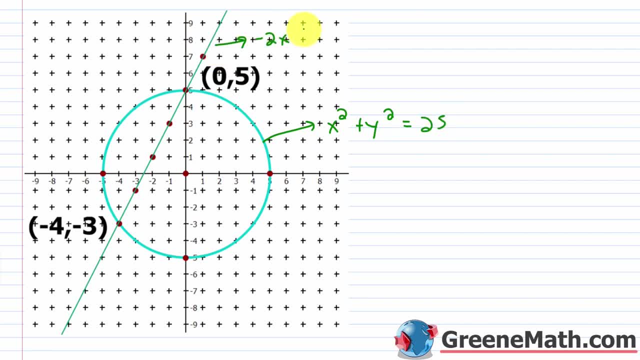 We see we have our line. Again. this is negative. two x plus y is equal to five, And we can see that this point right here, zero comma five exists on both of the graphs. right, It exists on the graph of the line and it exists on the graph of the circle, So we can see that it satisfies both. 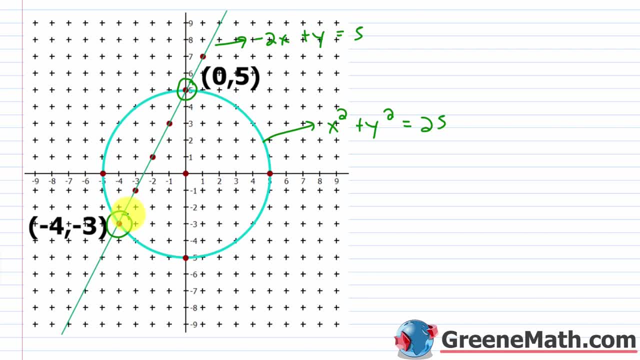 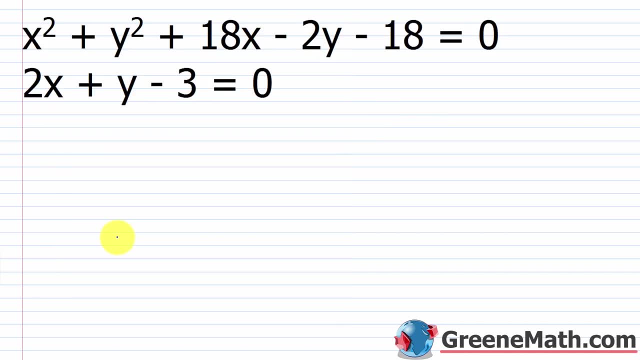 equations, And the same thing happens here: Negative four comma, negative three. this point is on the graph of the circle. It's also on the graph of the line. For the next example, we'll see the exact same concept. We have a second degree equation and a linear equation. So we have x. 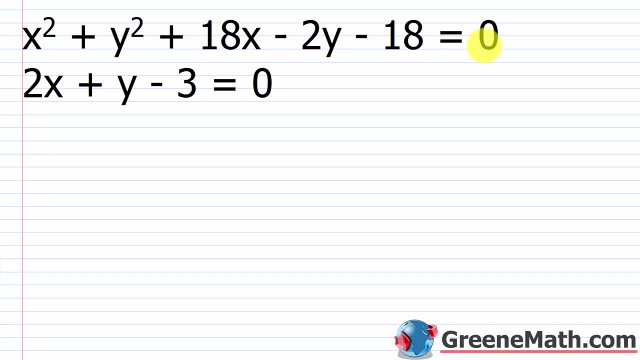 squared plus y, squared plus 18, x minus two, y minus 18 equals zero. We have two x plus y minus three equals zero. So this is equation one And this is equation two. Now what I'm going to do again is solve the linear equation, equation two, for one of the variables. In this case, I'm just going to 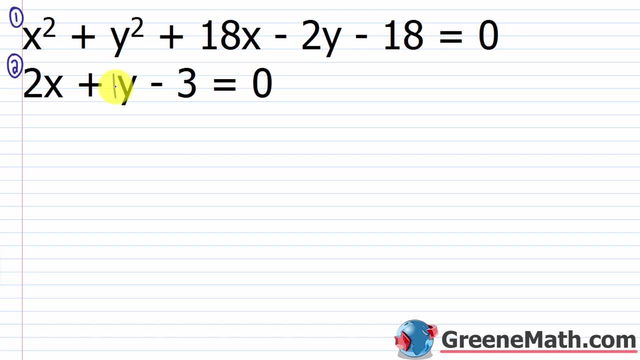 solve it for y again, because there's a nice easy coefficient of one there by y. So I would subtract two x away from each side And I would add three to each side And that would give me y is equal to negative, two x plus three. 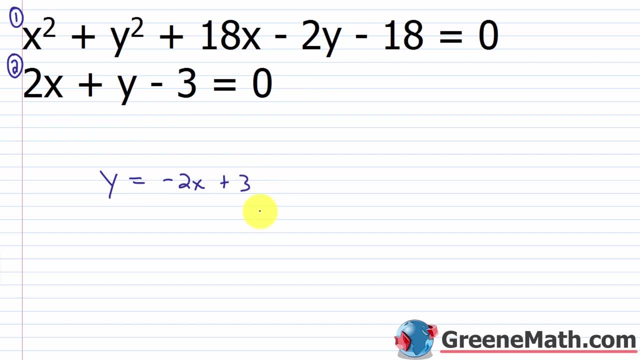 So once I've done that, I can then plug in for y in this equation up here. So I'm going to plug in here, but now also here. So this problem is going to be a little bit more tedious because there's more stuff to do. So I'll end up with what I'll have: x squared plus again plugging in for y. 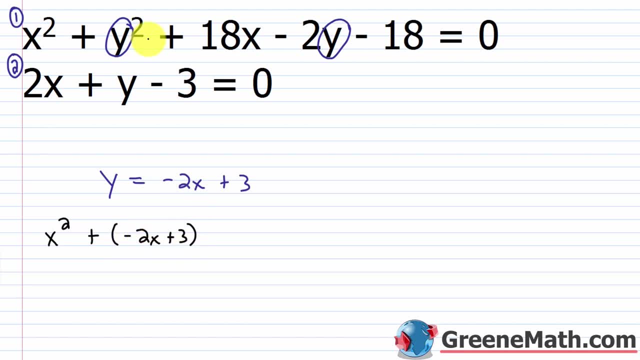 I'll have this quantity negative two x plus three. This is squared plus 18 x, then minus two times again I'm plugging in for y. So this negative two x plus three and then minus 18.. Okay, and then? 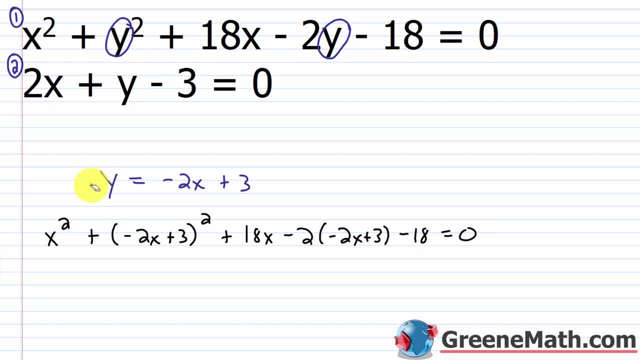 this equals zero. All right, so now we have that out of the way. Let me erase this, And then I'll just slide this up. All right, so now we just have some simplifying to do So. we have x squared plus. I use my special. 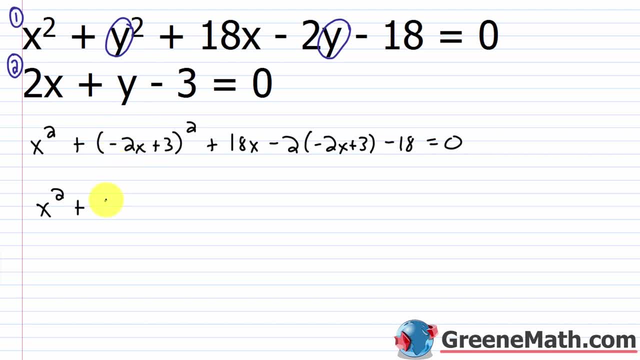 products formula. there I would square negative two x, that would be four x squared. And then I would do two times negative, two x times three. If you think about two times negative two, that's negative four. negative four times three is negative 12.. So you'd have negative 12 times x. 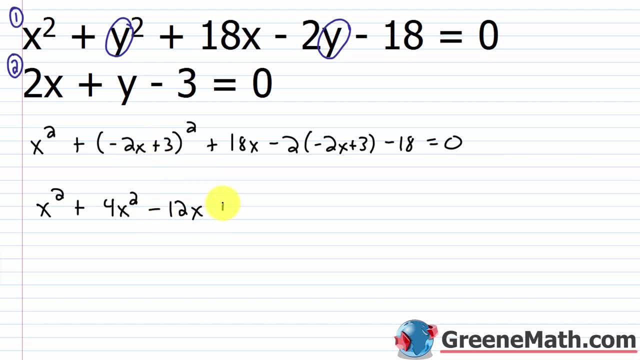 or minus 12 x, And then I'd have three squared, which would be nine, so plus nine. then I have this negative two to each term here. So negative two times negative two x is plus four x, And then negative two times three would be minus six, And then we have minus 18.. And then this equals zero. 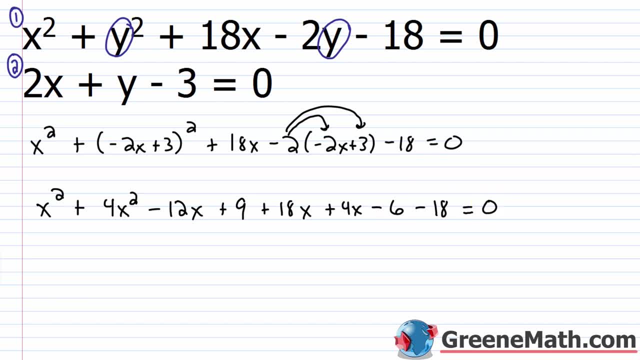 All right. so what can we combine here? Well, these are like terms, these are like terms, And then these are like terms there. All right, so x squared plus four x squared would be five x squared Plus 18: x is six x, And then six x plus four x is 10 x. so plus 10 x, Then we have nine minus six. 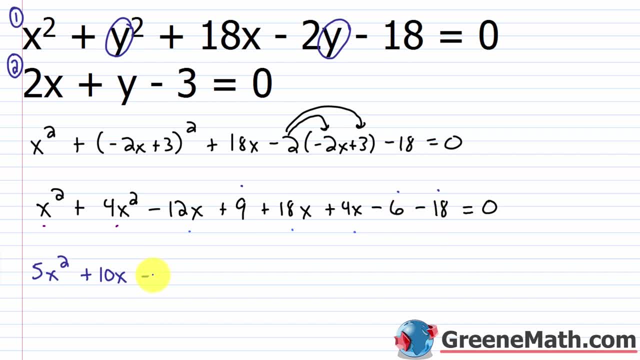 which is three, And then three minus 18 would be negative 15. And then this equals zero. All right, so let me erase everything. Let's slide this up. So most of you will notice that you could divide both sides of the equation by five here, And that'll make the numbers. you're working with a. 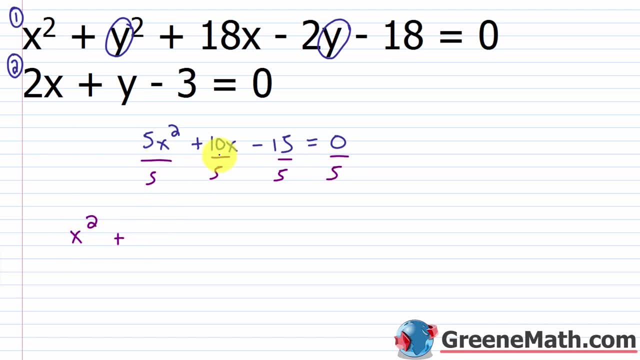 little smaller. So you'll have x squared plus 10 over five squared, And then you'll have six x squared over five is two. So two x and then minus three, and this equals zero. So I can solve this by factoring. I know the left part here would factor into what. So give me two integers that sum to two. 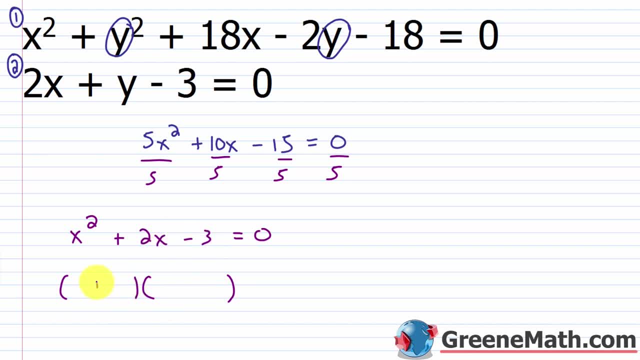 and multiply together, give me negative three. Well, I could do plus three and minus one. Three minus one is two. Three times negative, one is negative three. So x plus three and x minus one, and this equals zero. All right, let's erase all this And we'll bring this up. 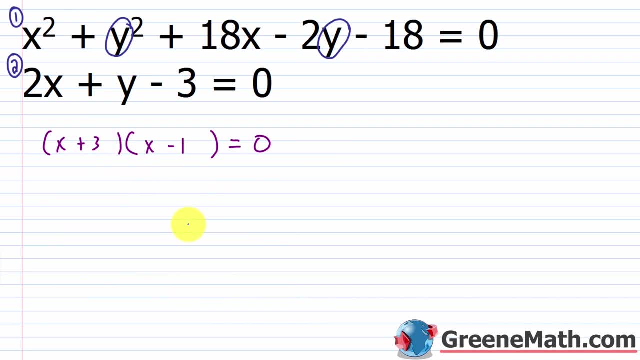 So I'm going to set these two factors equal to zero and I'm going to solve: I'll have x plus three is equal to zero or x minus one is equal to zero. Of course, these are very easy to solve. I just 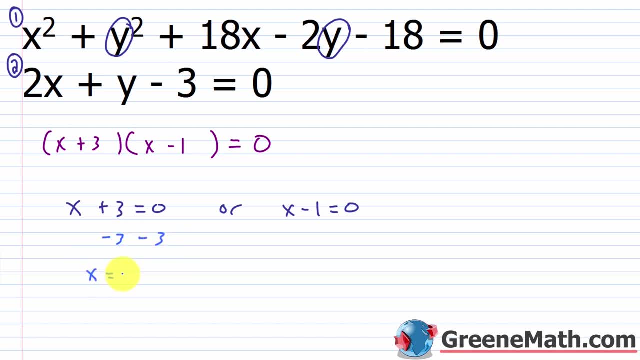 subtract three away from each side of the equation. here I get x equals negative three. Over here I add one. each side of the equation, I get x is equal to one. So I know that we have x equals negative three. and then we have x equals one. 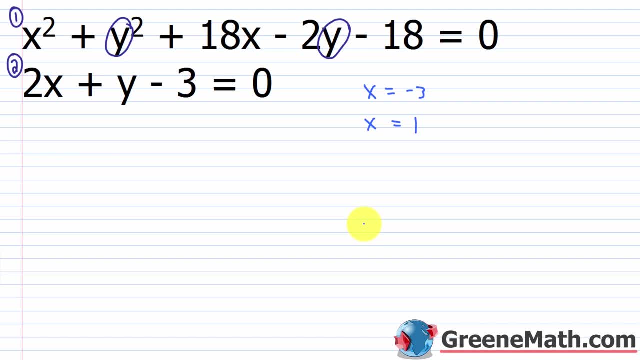 So let's erase everything. And again, I just want to plug in to one of the equations and see what my value is for y for each given x value. Now the linear equation is much easier to work with. If you want to plug into equation one, you can. I recommend you end up doing that. 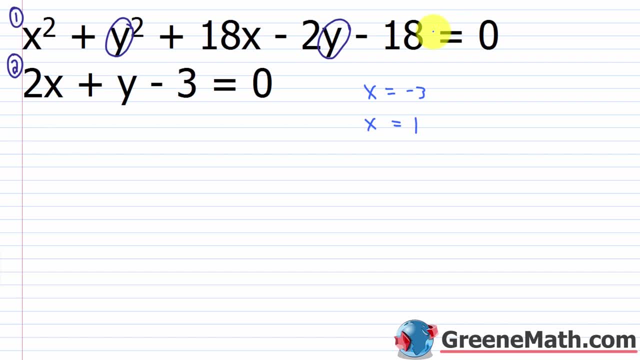 just as a check with the solution that you get. So if x is negative three, I'd have two times negative three plus y minus three equals zero. This would be negative. six plus y minus three equals zero. Negative six minus three would be negative nine. So I would have y minus nine, equals. 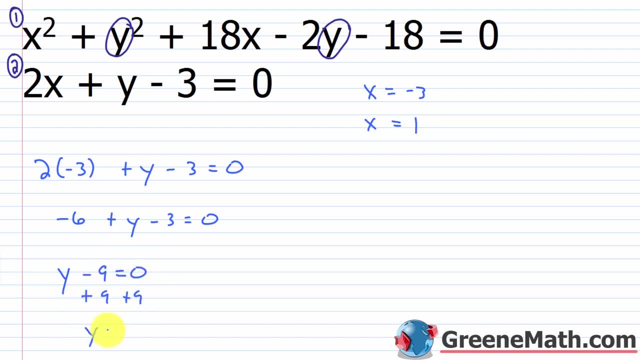 zero. Add nine to each side of the equation I get y is equal to nine. So if x is negative three, y is equal to nine. All right, let's try the other scenario now. So what about when x is one? So two times one is two, So you'd have two minus three. 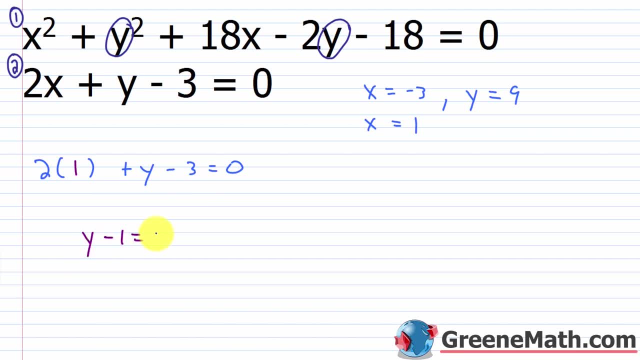 which would give me negative one. So you'd have y minus one. one equals zero. Add one to each side of the equation You get y is equal to one. So as our solution set goes, we'll have the order pair: negative three comma nine. 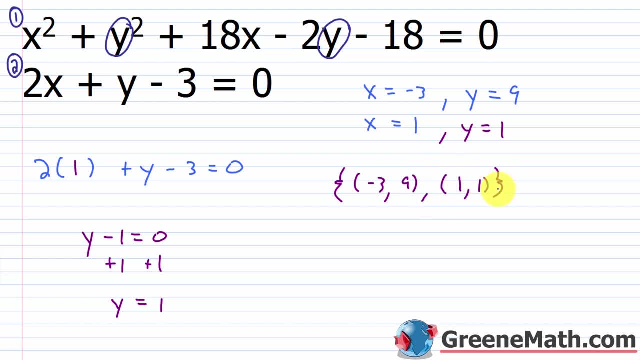 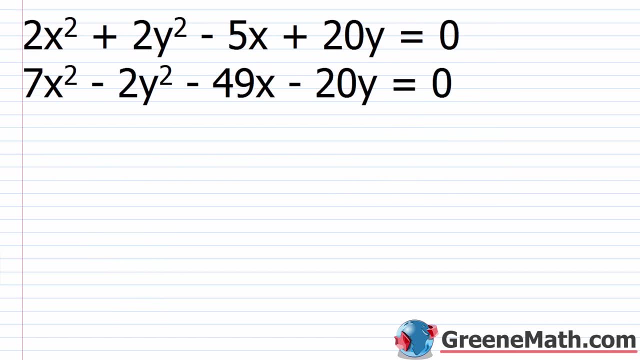 We'll have the order pair: one comma one. Now I'm not going to go through and check these, but I recommend that you do. I already know they work, because when I set up these problems I did check them. All right, let's look at a different scenario now. So when you see two 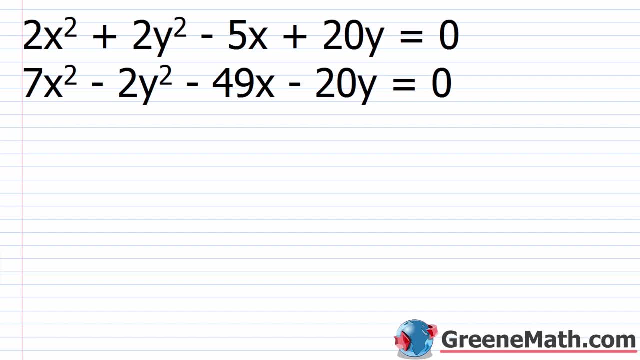 second degree equations. what you want to use now is a two second degree equation, So you want to use elimination. So let's say we see something like two x squared plus two y squared minus five x plus 20 y equals zero. And then seven x squared minus two y squared minus 49 x minus 20 y equals 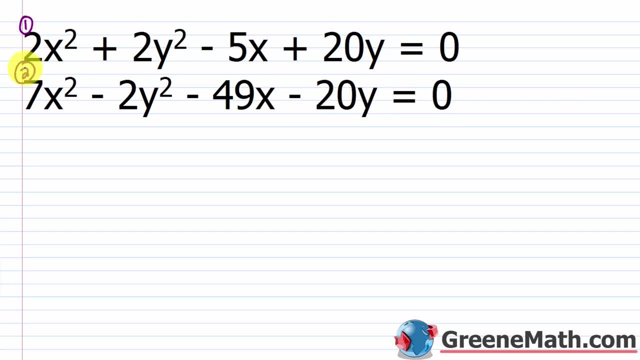 zero. So I'm going to call this equation one and this equation two. Now, most of the problems you're going to see in an algebra, two course, we'll set up to where you can just add the equations right away and you'll have one of the variables be eliminated. So if I add equation one, 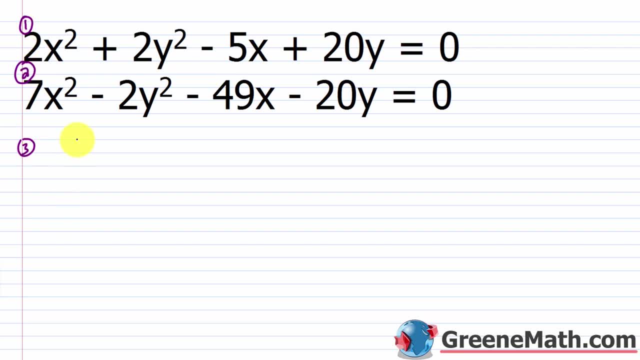 and equation two together, that'll give me equation three. So two x squared plus seven x squared would give me nine x squared. Two y squared minus two y squared would give me zero y squared. or we could just say zero And then negative: five x minus 49 x. 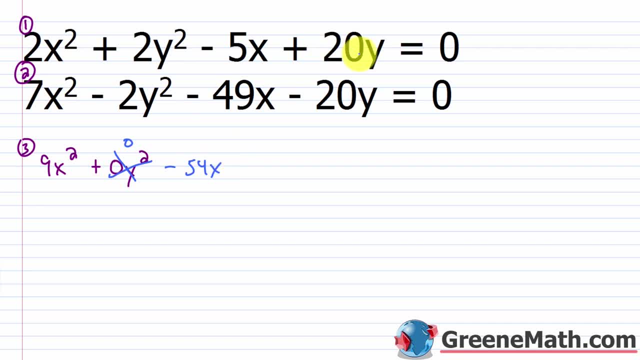 we'll say that's minus 54 x, And then 20 y minus 20 y. let's say this is plus zero y, or again this is zero, And then this equals zero. So what I'm left with now is nine x squared. 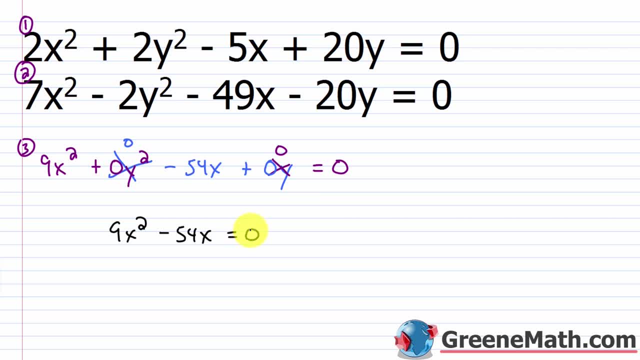 minus 54 x, and this equals zero. So this is something I can solve very quickly using factoring. I can factor out a nine x and I'll have x minus six inside the parentheses. This equals zero. Let me erase all of this. We don't need any of this information anymore And I will. 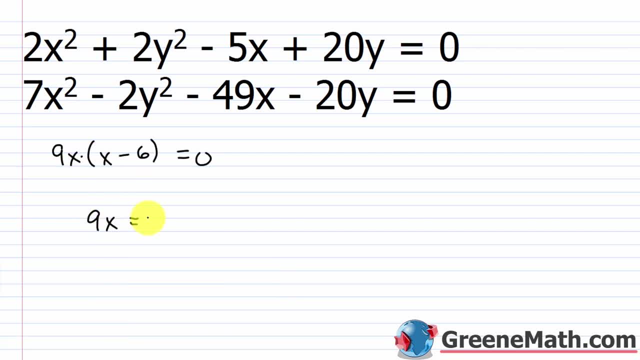 just scooch this up: Nine, x is a factor, So I'm going to set that equal to zero. Then, or the quantity x minus six, that's a factor, I'll set that equal to zero. Very, very easy equations to solve. Divide both sides of the equation by nine. here We see x is equal to zero. Here I can. 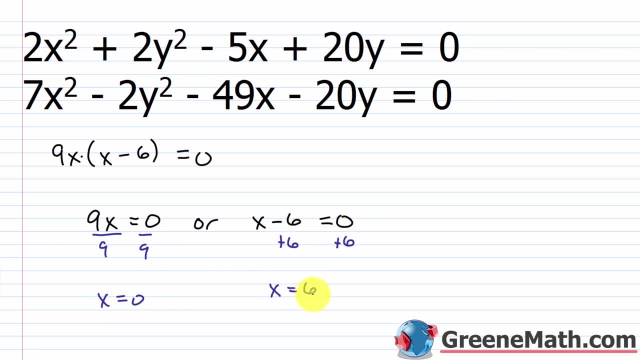 add six to each side of the equation, I'll see that x is equal to six. So let me erase everything. And the substitution part here is a little bit more tedious than it was before because you don't have a linear equation anymore. All right, so let's see what happens when x equals zero. So 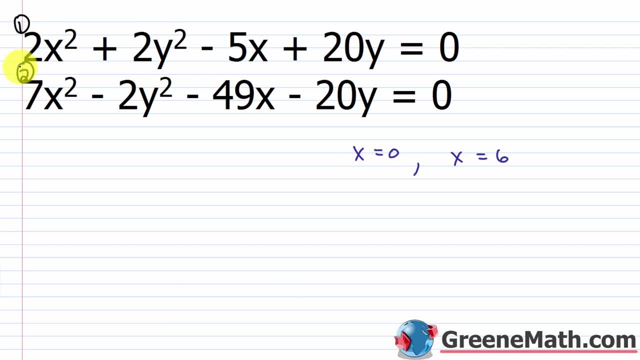 I'm going to go back and label this as one and two and I'm going to plug in a zero for x in equation one. So two times zero squared plus two, y squared minus. five times zero plus 20, y is equal to zero, All right. 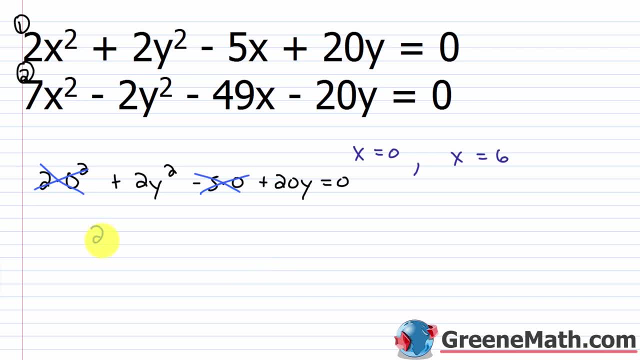 so this is gone and this is gone. So basically what I have is two y squared plus 20. y is equal to zero. Now what I can do is I can divide each side of the equation by two. You can make those numbers smaller So that cancels. I'll have y squared plus. 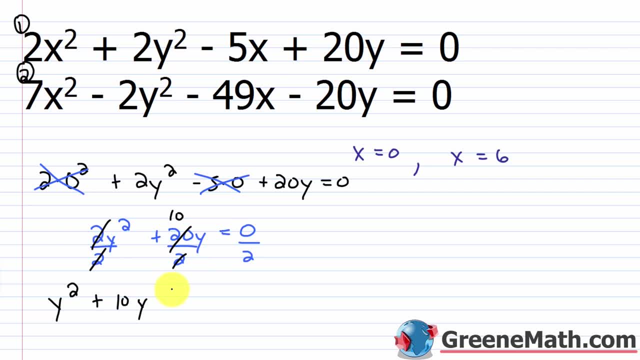 this cancels with this and I have 10.. So 10 y and this equals zero. Let me erase all this And we'll slide this up. Let's get some room. I can solve this by factoring. If I factor out a y, 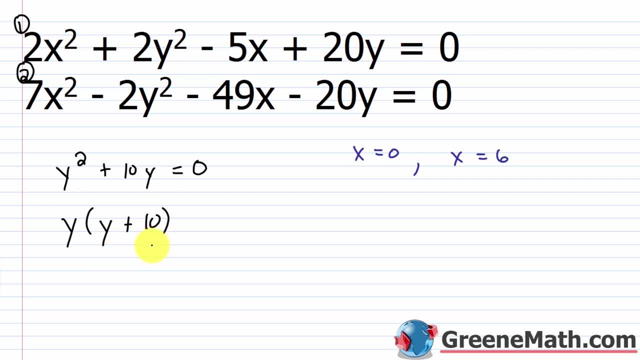 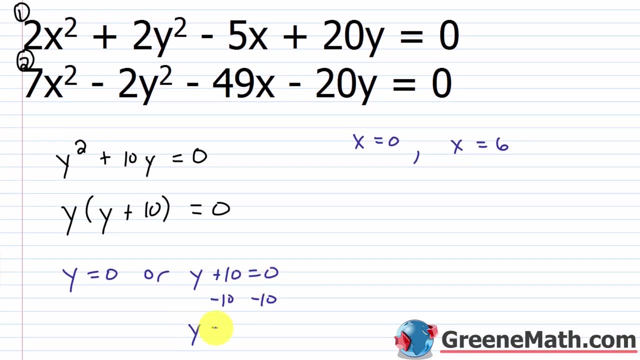 I would have y plus 10 inside the parentheses. This equals zero. So one of the solutions here would be that y is equal to zero. The other solution would be: y plus 10 equals zero. We know we could subtract 10 away from each side of the equation. That would give me that y is equal. 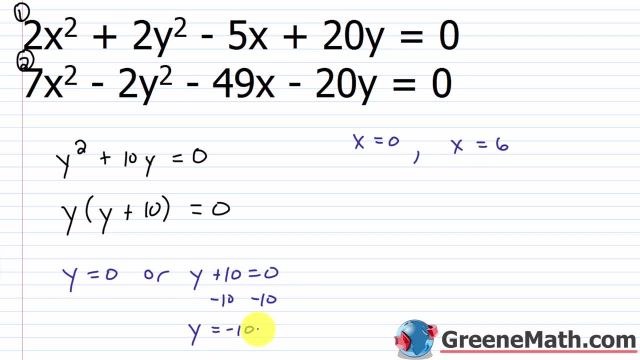 to negative 10.. So the solution here: when x equals zero, there's two different y values. that's kind of partnered up with that. So in other words, you'd have the ordered pair zero comma zero, but you'd also have the ordered pair zero comma negative 10.. So let me kind of write this over. 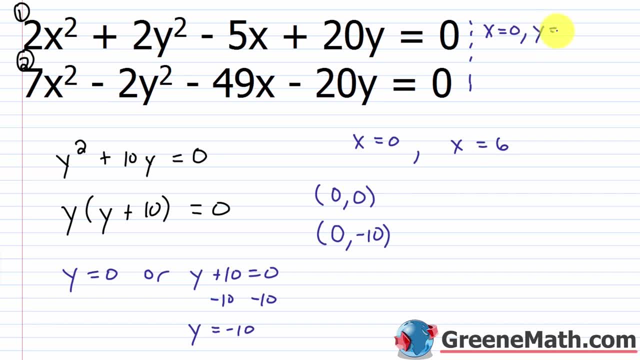 here: x equals zero, y equals zero. You'd also have x equals zero, y equals negative, 10.. Now let's see what happens when x equals six. So if x equals six, again I'm just going to plug into equation one. The numbers are a little. 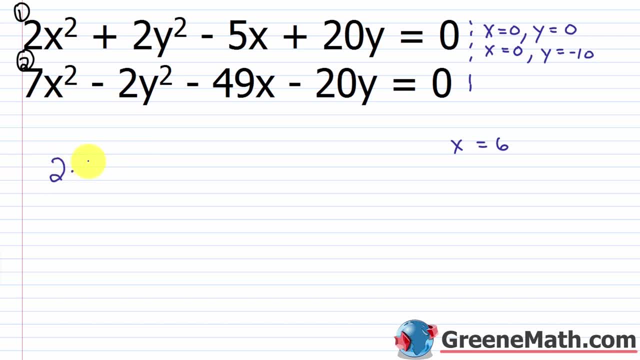 smaller so it's easier to work with. So we'd have two times six squared plus two y squared minus five times six, plus 20 y equals zero. So six squared is 36.. So two times 36 is 72.. Plus two y squared negative. five times six is negative 30.. So minus 30, then plus 20 y. 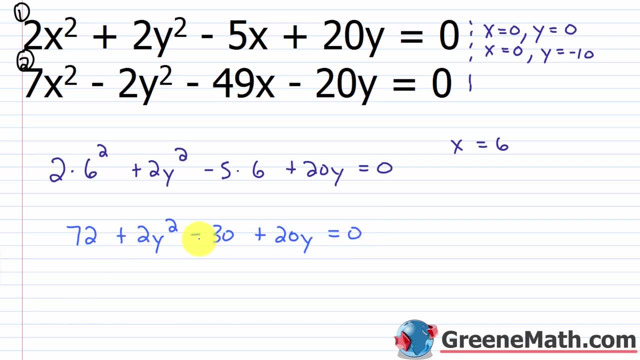 and this equals zero. So what is 72 minus 30?? It's going to give us 42. So I can just get rid of this and just put this as 42 over here. Then I can subtract 42 away from each side of the equation. 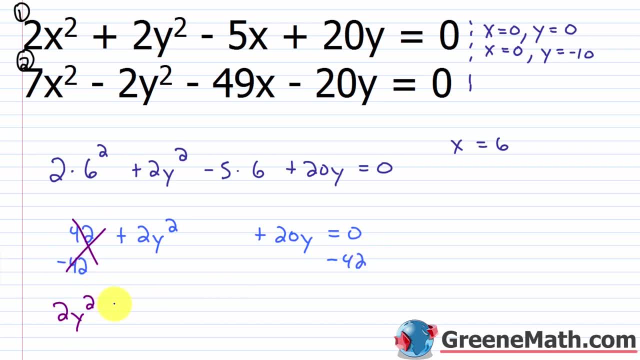 So this is going to go away. I'll have two y squared plus 20. y is equal to negative 42.. All right, so let's erase all this And I'll bring this back up. All right, so I'm going to divide each side of the equation by two. 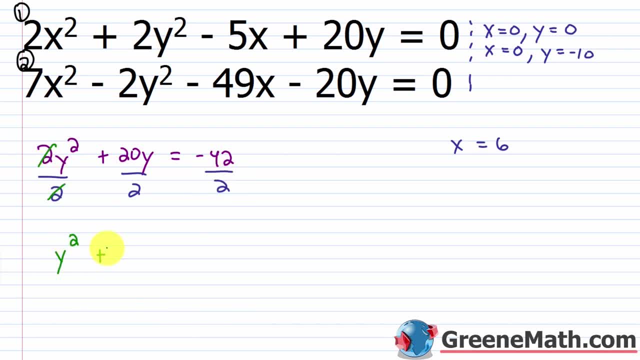 So this will cancel with this and I'll have y squared. Then plus this will cancel with this and I have 10.. So plus 10 y, This equals this cancels with this. So I know it's negative 42. 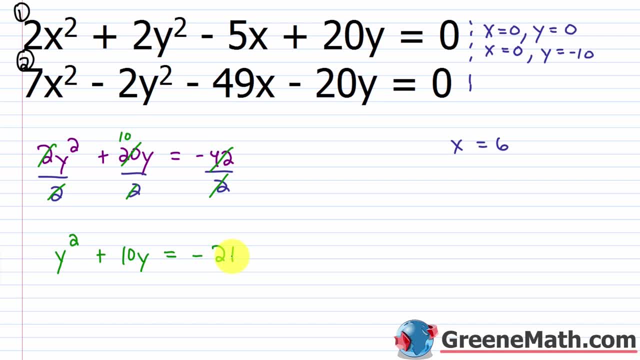 divided by two is 21.. So y squared plus 10 y equals negative 21.. So what I can do there? I can add 21 to each side of the equation. I'll have y squared plus 10. y plus 21 equals zero. 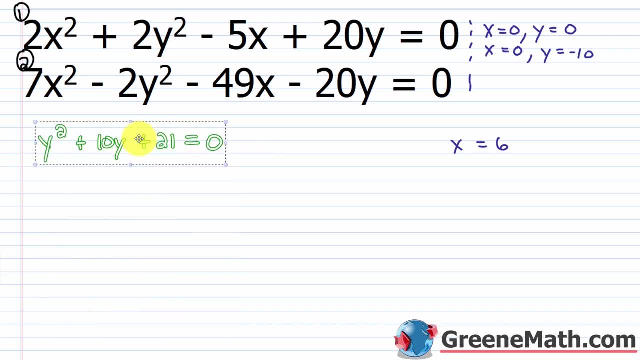 Now, this is factorable, so I can solve it that way. Let's just slide this up, All right. so what is this factor into? on the left side, Give me two integers whose sum is 10 and whose product is 21.. It's easy: seven and three. 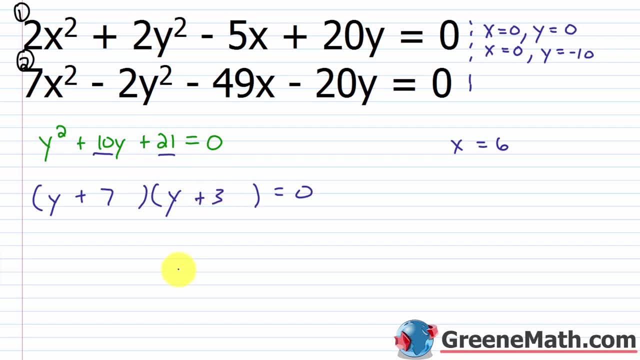 So y plus seven and y plus three. So we know the solutions here. We would set y plus seven equal to zero. So we'd set y plus seven equal to zero. We know that this solution. here We would set y plus seven equal to zero. 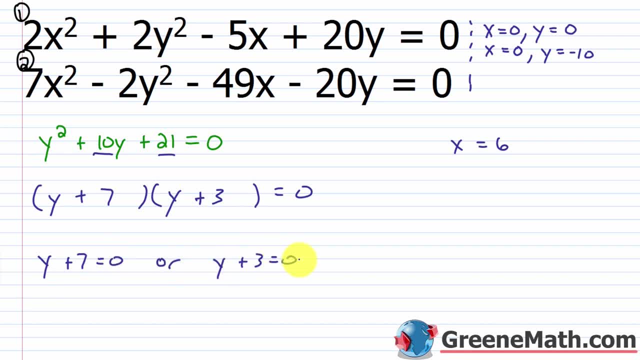 Then we would also set y plus 3 equal to 0.. Over here I would subtract 7 away from each side of the equation, I would get y is equal to negative 7, or over here I'd subtract 3 away from each side of the equation and I'd 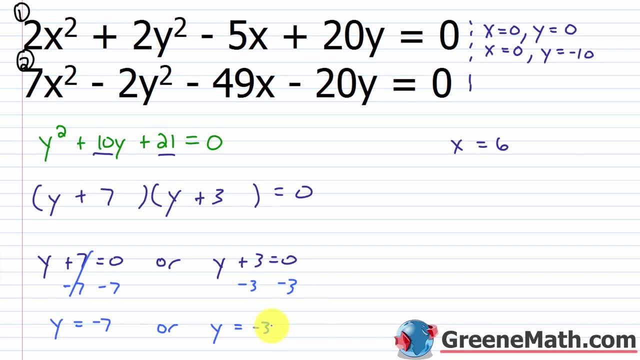 find that y is equal to negative 3.. So if x is 6,, y could be negative 7,. or if x is 6,, y could be negative 3. So you have x equals 6, y equals negative 7,. you have x equals 6, y equals negative. 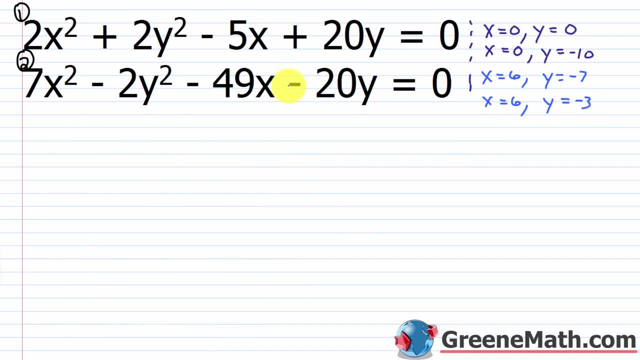 3. Alright, so let's erase all this. Alright, so our solution set here: we're going to have the ordered pair, we're going to have the ordered pair, we're going to have the ordered pair, and then we'll have the ordered pair. 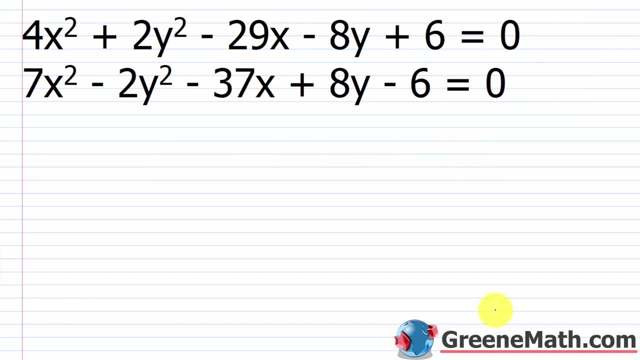 Alright, let's take a look at one more of these. So we have 4.. 4x squared plus 2y squared minus 29x minus 8y plus 6 equals 0.. We have 7x squared minus 2y squared minus 37x plus 8y minus 6 equals 0.. 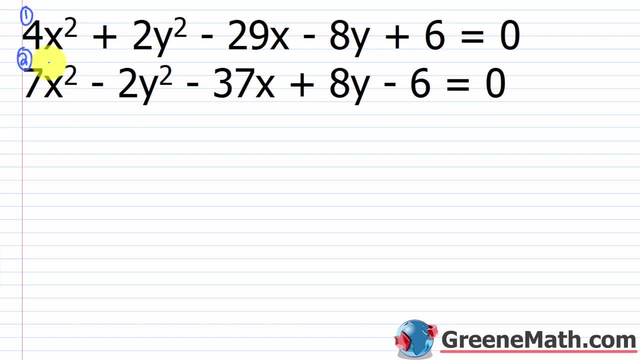 So let's call this equation 1 and this equation 2.. Two second degree equations and again in your book or whatever you're using to kind of study this, especially in Algebra 2, they give you these easier problems where it's. 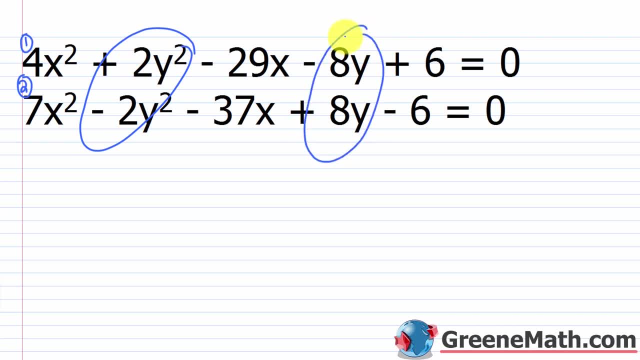 kind of set up where these are opposites and these are opposites. So I can add the two equations right now And I can basically eliminate y. So we're going to use elimination. 4x squared plus 7x squared for equation 3 would give me 11x squared. 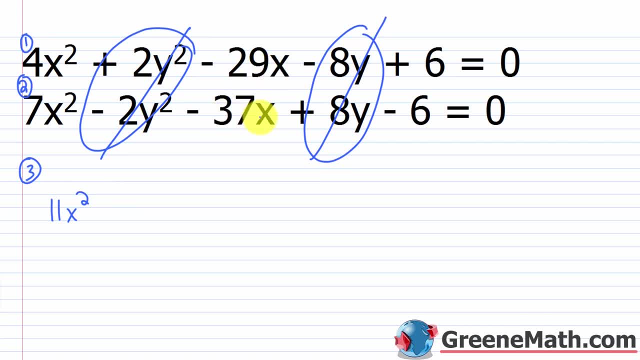 These would be eliminated. These would be eliminated. Negative 29x plus negative 37x would be negative 66x, And then 6 minus 6, that's gone. So this just equals 0.. So the first thing is I can divide both sides of this equation by 11 and make everything. 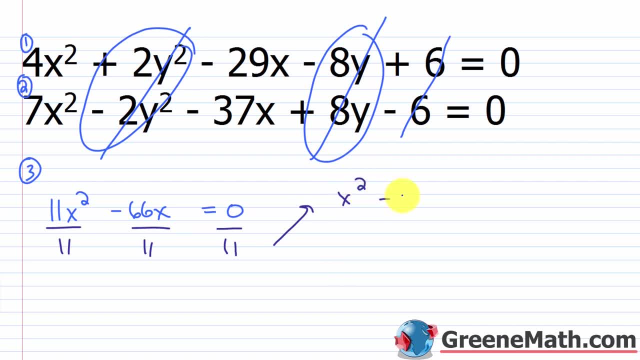 smaller. This would be: x squared minus 6x equals 0.. So let me erase this and I'll slide this over. Of course we can solve this guy by factoring. If I factor out an x, I'll have x minus 6 inside the parentheses. 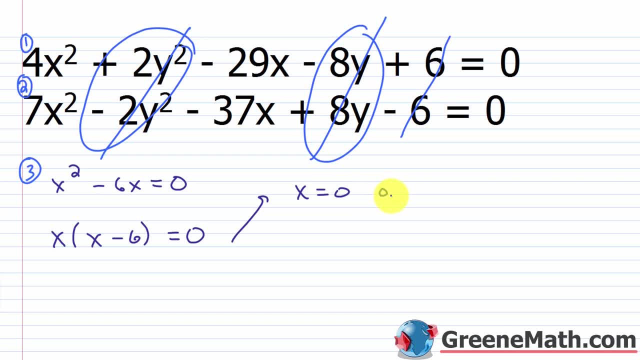 We set this equal to 0. We say that x could be 0 or x could be what? If I set x minus 6 equal to 0, I know the solution would be positive 6. So x could be 0.. 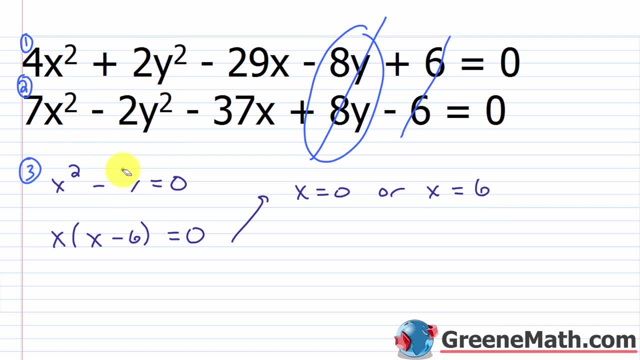 Or x could be 6.. All right, So let's erase everything And I'll keep this here for now, kind of slide it over just a little bit. So what happens when x is 0? Let's just pick, I don't know. equation 1 looks a little bit easier. 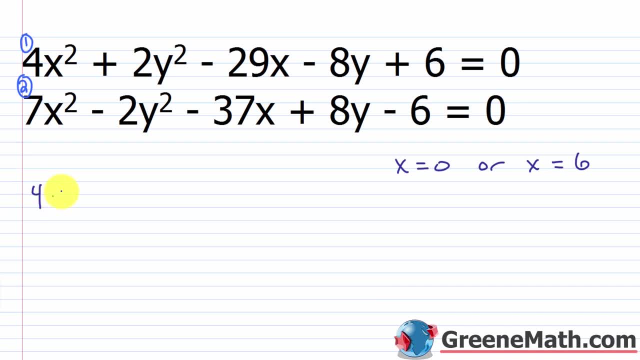 Let's pick equation 1 to work with. So if x is 0, we'll have 4 times 0 squared plus 2y squared minus 29 times 0 minus 8y plus 6 equals 0. So we know that this is going to go away and this is going to go away. 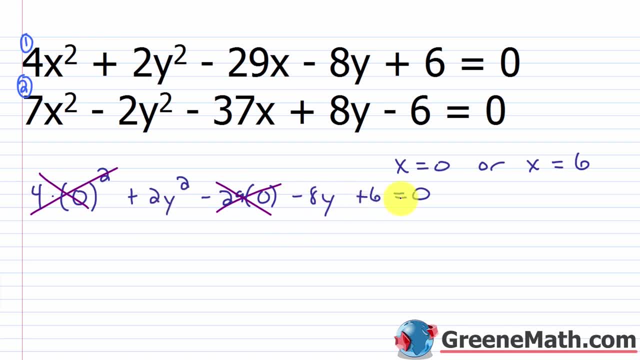 I'll basically have: 2y squared minus 8y plus 6 equals 0.. Now I can divide each side of the equation by 2 and make that a little easier. So y squared minus 4y plus 3 equals 0.. 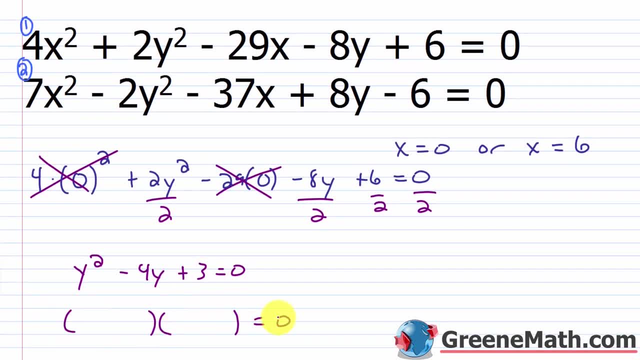 I can factor this y and y. So give me two integers whose sum is negative 4 and whose product is 3.. You could do negative 3 and negative 1.. So minus 3 and minus 1.. So I could set each factor here equal to 0. 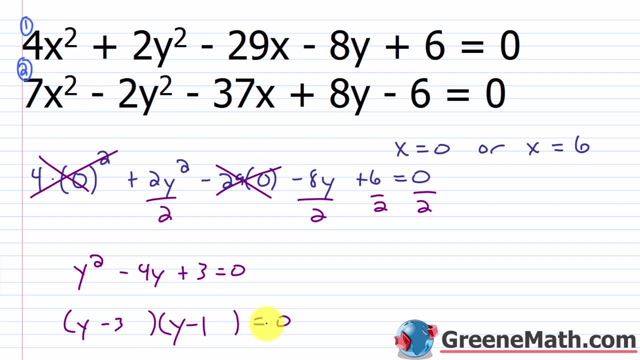 So you'd have y minus 3 equals 0, and then you'd have y minus 1 equals 0. Of course, the solution to this one would be that y equals 3.. The solution to this one would be that y equals 1.. 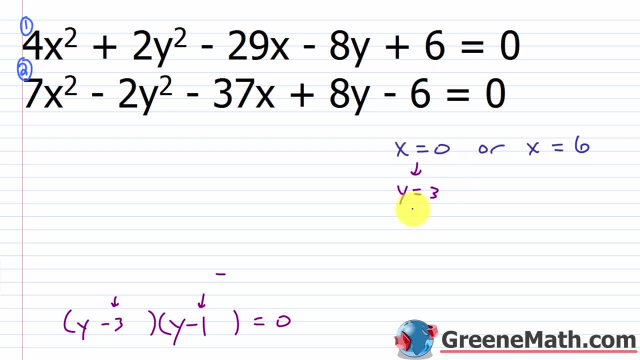 If x is 0, y is equal to 3 or it's equal to 1.. So we're going to set this up over here and I'll just say We have the ordered pair 0, 3.. We also have the ordered pair 0, 1.. 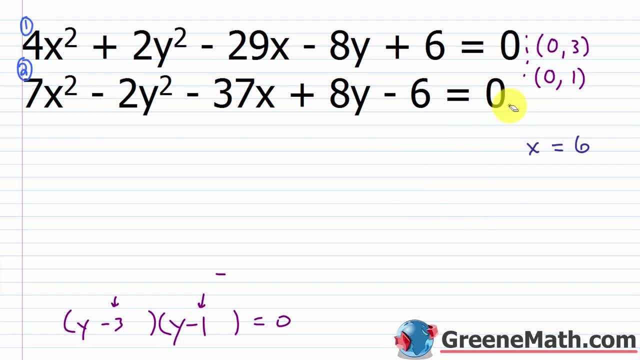 All right. so let's get rid of that. All right. now let's see what happens when x equals 6.. So I'm going to go into equation 1 again. We'll say: 4 times you'll have 6 squared plus 2y squared minus 29 times 6 minus 8y plus. 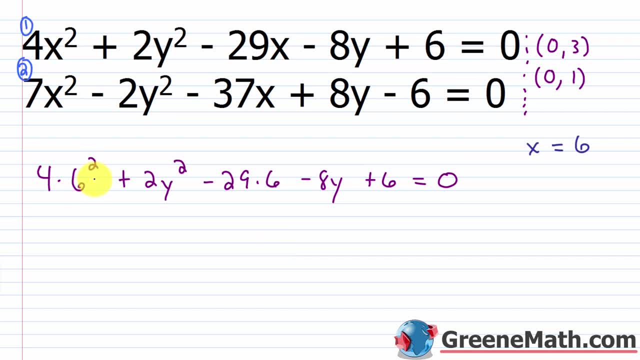 6. And this equals 0.. All right, So 6 squared, we know, is 36.. 4 times 36 is 144.. So let me erase this and just put 144.. 29 times 6 is 174.. 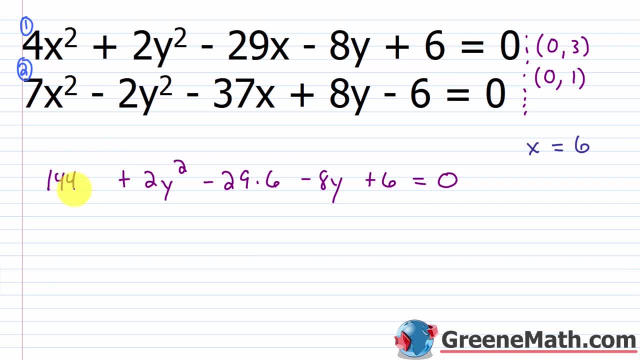 So let me put minus 174. And we know that 144 minus 174 is negative 30. So let me just put negative 30, and then we're adding 6, so that's negative 24. So I'll put negative 24 back here. 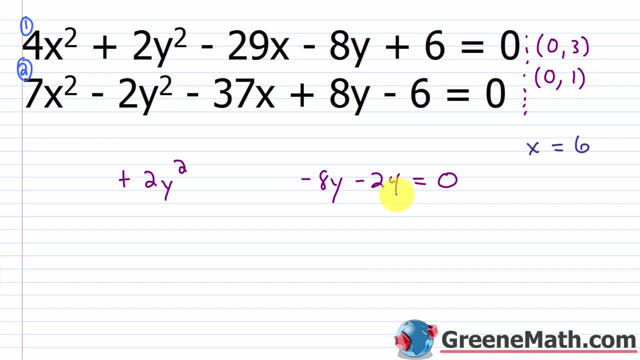 All right. So what we're left with is 2y squared minus 8y minus 24 equals 0. So let me erase this and we'll kind of scooch this down Now. one thing I can do is I can divide everything by 2.. 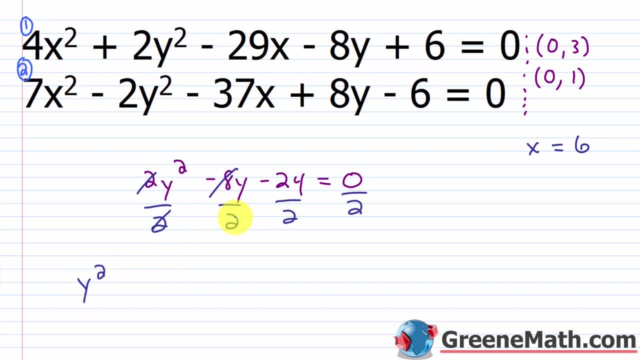 So this would cancel. I'd have y squared. This would cancel with this and give me negative 4.. So I'd have minus 4y. This would cancel with this and give me negative 12.. So minus 12 and this would equal 0.. 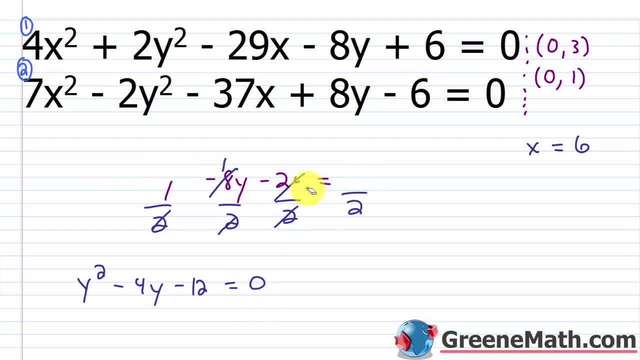 Now can I solve this by factoring? Yes, I can. Let me erase this real quick and I'll slide this guy up So I can factor the left side here. This is y, This is y. Give me two integers that sum to negative 4 and multiply together to be negative 12.. 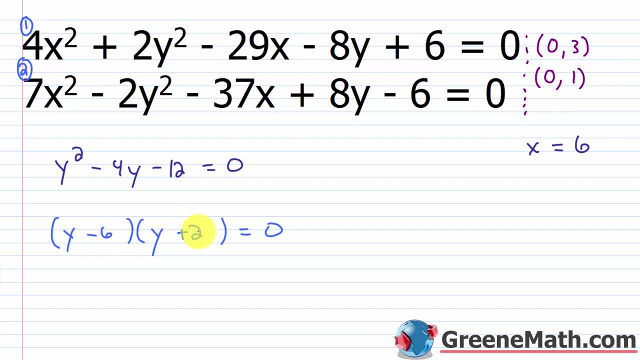 Well, of course you could do negative 6 and positive 2.. So we know the solutions here would be that y equals 6 or y equals negative 2. Right, So these factors equal to 0. So y equals 6 or y is going to equal negative 2.. 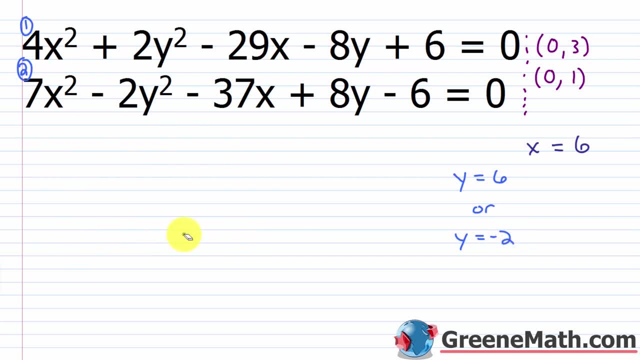 So let's erase this. And so our ordered pairs would be 6 comma 6 and then also 6 comma negative 2.. So in solution set notation we'll say we have 0 comma 3 as a solution, 0 comma 1 as. 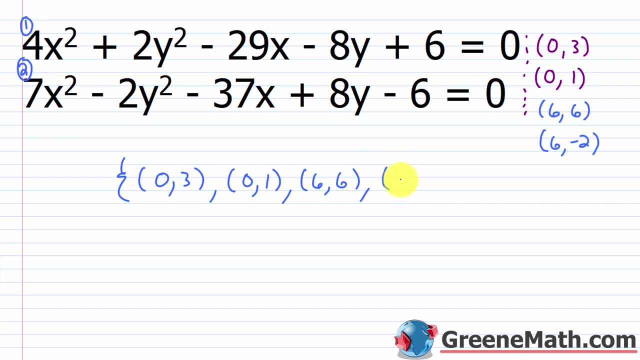 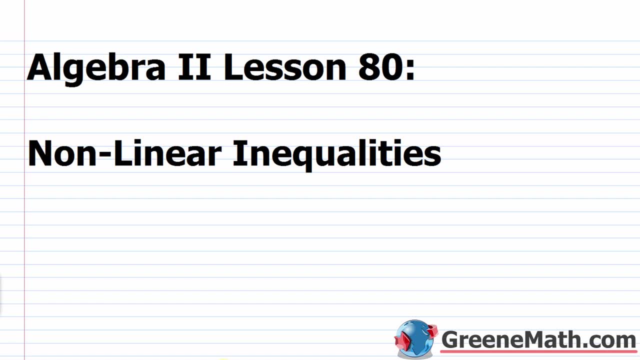 a solution: 6 comma 6 as a solution and 6 comma negative 2.. So we've got 6 comma negative 2 as a solution. Hello and welcome to Algebra 2, Lesson 80. In this lesson we're going to learn about nonlinear inequalities. 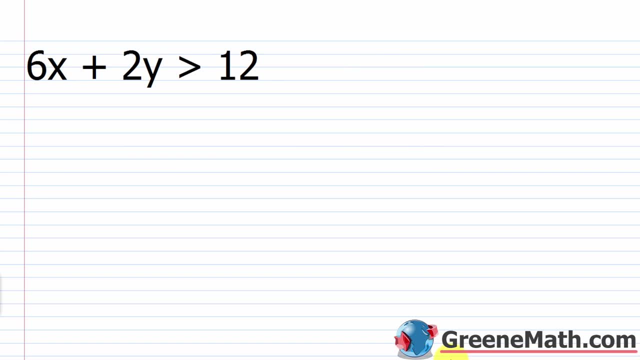 So hopefully at this point everybody knows how to solve a linear inequality in two variables and also how to solve a system of linear inequalities in two variables. I just want to take a few minutes here and review how to do this type of problem. Pretty much everything we're going to do in this problem is going to carry forward into 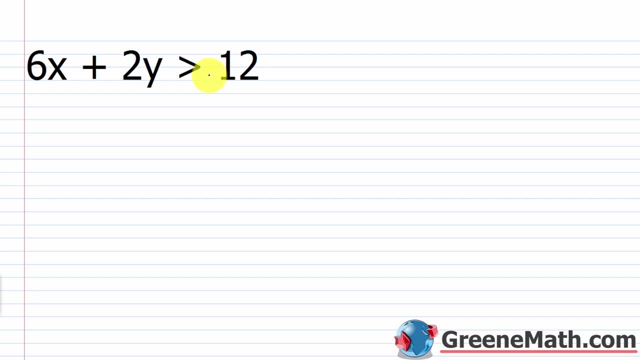 solving a nonlinear inequality, and then also the same concepts are going to be used when we solve a system of nonlinear inequalities. If we have a problem like 6x plus 2y is greater than 12, what's the first thing we want to? 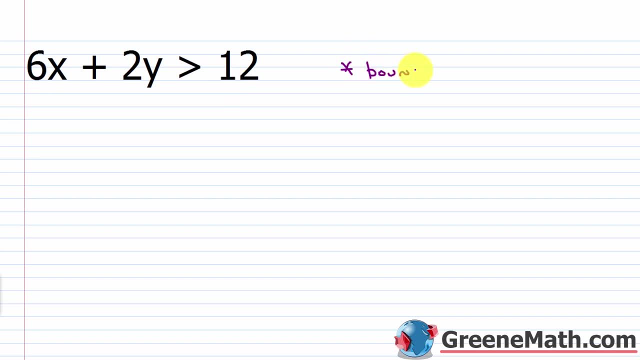 do? We want to find the boundary. We want to find the boundary And in this case it's going to be a boundary line. But later on, if we're working with nonlinear inequalities, we won't have a boundary line. The boundary will be a different shape. 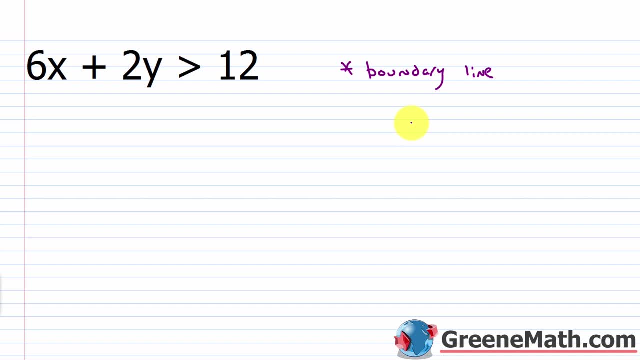 But the boundary is an important concept to get down When you're on the coordinate plane. the boundary is going to separate the coordinate plane into two regions. One region is the solution region, So all the points there will satisfy the inequality. The other region, on the other side of the line, is going to be in the non-solution region. 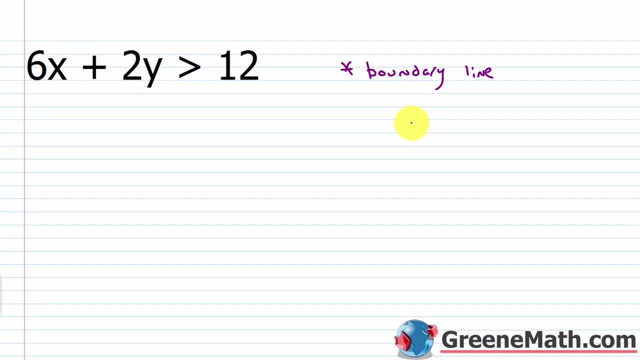 So every point there will not work or will not satisfy the inequality. So you're either in the solution region or you're in the non-solution region. It's one or the other. Now the boundary line. there's two scenarios. There's one where the boundary line is included in the solution set. 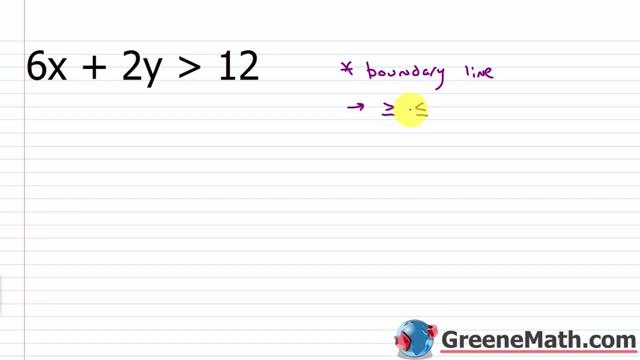 So when it's included is when we have a non-strict inequality, So basically a greater than or equal to, or less than or equal to, And for this we get a solid boundary line. Now, if it's a different shape you're working with, maybe a circle or an ellipse or whatever- 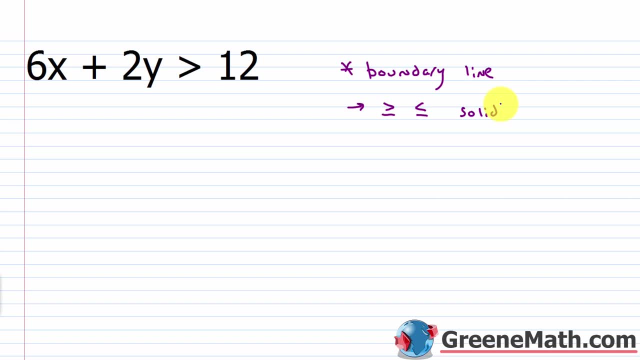 it is. we wouldn't say solid line, We'd say solid circle, or solid ellipse, or solid hyperbola, you know so on and so forth. Then the other scenario is: if you have a strict inequality, So if you have something that is strictly greater than or strictly less than you get. 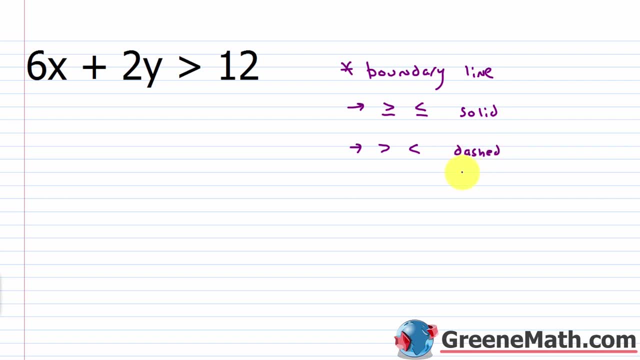 a dashed or broken up line to show that the boundary line is not part of the solution. So how do we get the boundary line or the boundary in general? Essentially, we look at the inequality symbol and we replace it with equals. So I would have: 6x plus 2y is equal to 0.. 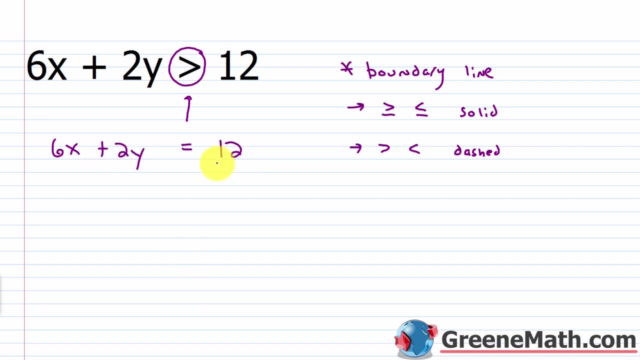 I can easily solve this guy for y and graph the resulting line. So let's subtract 6x away from each side of the equation. That'll give me 2y is equal to negative 6x plus 12.. Let me divide both sides of the equation by 2.. 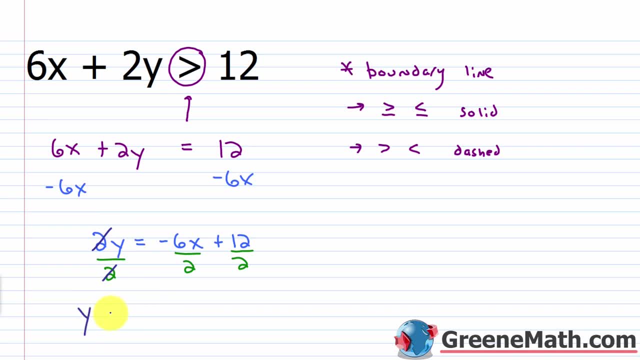 And we'll see that this will cancel with this and I'll have y. by itself, This is equal to negative. 6 over 2 is negative 3.. Then times x, Then plus 12.. 12 over 2 is 6.. 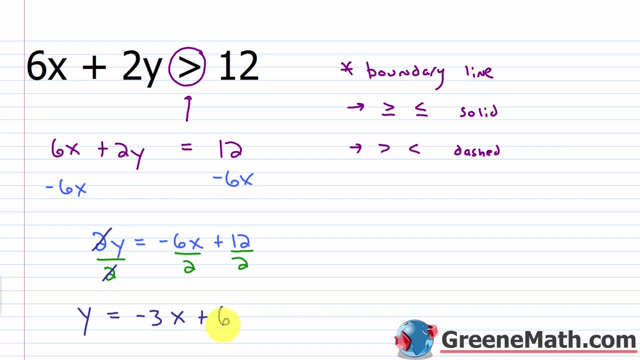 So this line right here is very easy to graph. It has a y-intercept of 0,, 6 with a slope of negative 3.. So the first thing we would do is graph this line, and we would graph it as a dashed line. 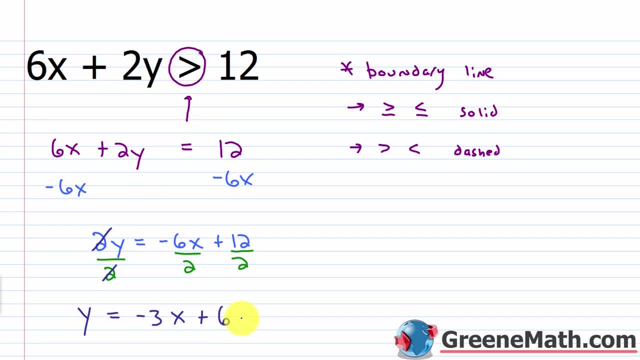 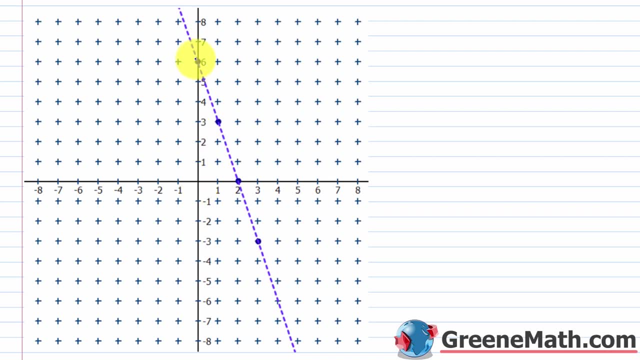 because we have a strict inequality here, strictly greater than. And so let's go to the coordinate plane, And I've pre-drawn everything today just to make it a little bit quicker for us. But again, the y-intercept occurs at 0, 6, which is right here. 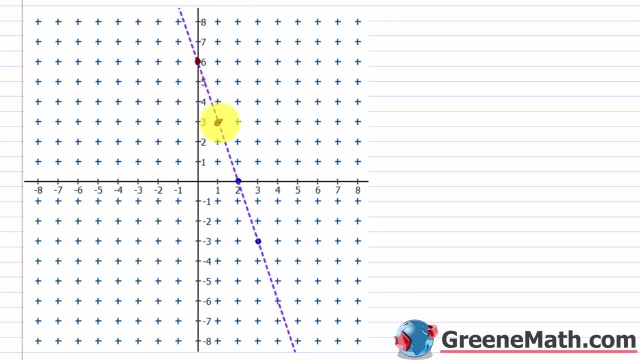 And the slope is negative 3.. So down 3 to the right 1, down 3 to the right 1, down 3 to the right 1, so on and so forth. We graph our line Again. this guy is dashed because it's not included in the solution. 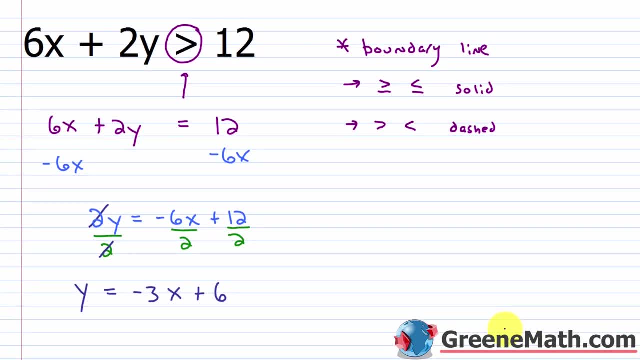 Now for the next part. you basically had two options: You could solve this guy for y and you could shade based on the direction of the inequality symbol, Or you could use a test point. So for today, we're going to go back to this test point method. 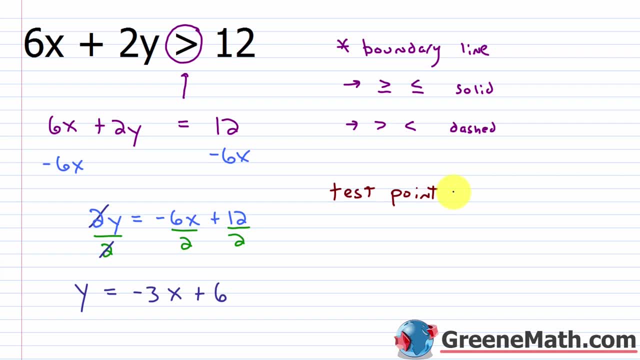 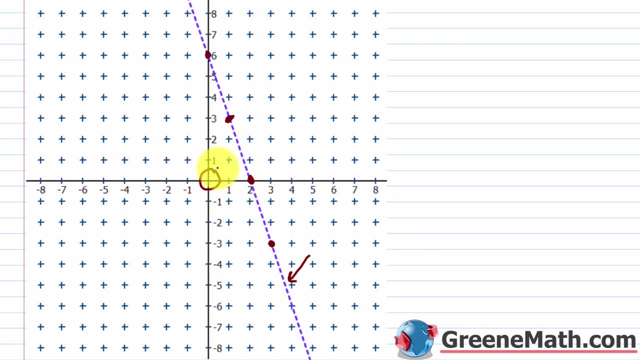 And with a test point I can choose any point on the coordinate plane that is not on the boundary line. So if I go back down I like to use 0, 0 because it's easy to work with. It's not on the boundary. 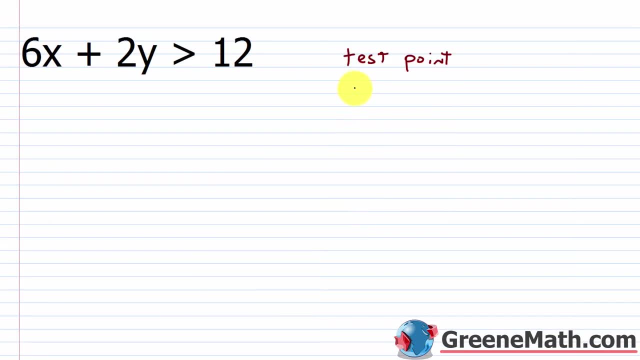 So let's go back up. So our test point is 0, 0.. So essentially, I'm going to plug in a 0 for x and a 0 for y, And what I want to know is: do I have a true statement? 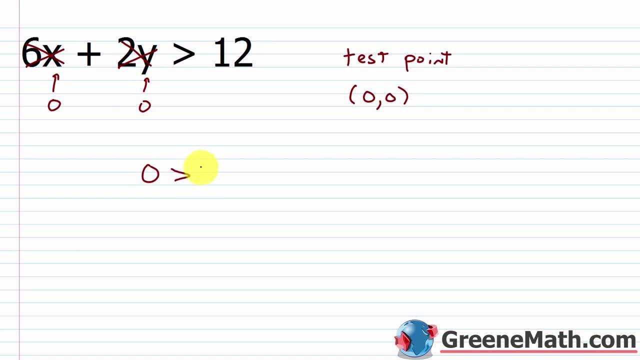 This would go away. This would go away. You'd have 0 is greater than 20.. You'd have 0 is greater than 12.. Is that true? No, it is not. This is false. Since 0, 0 does not work as a solution, we know it lies in the non-solution region. 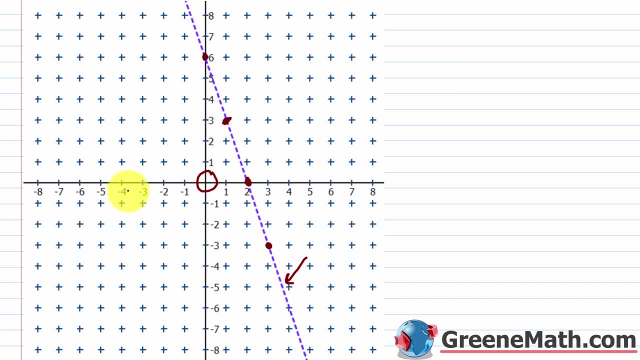 So you can think about this area right here, that's beneath or below the line, as the non-solution region. So this is the non-solution region. So everything on this side of the line does not work as a solution to the inequality. Well, anything on the other side of the line or above the line you could say, works as a 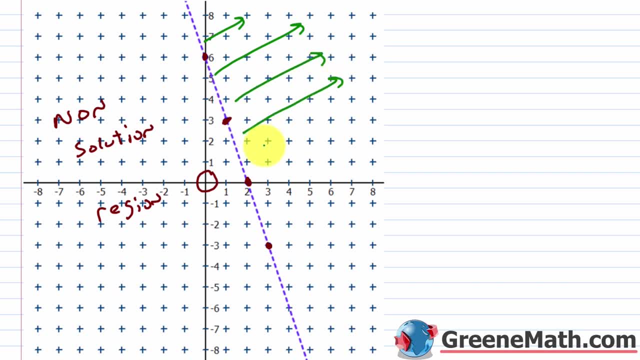 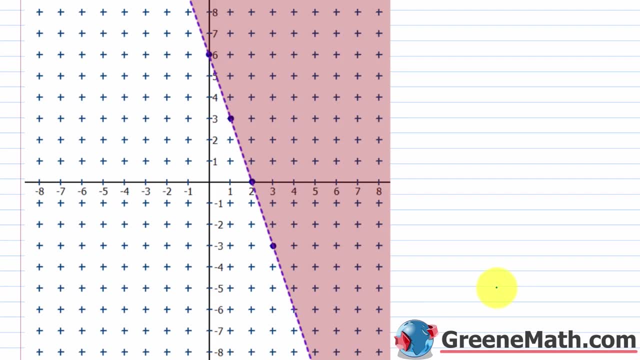 solution. So I would shade everything this way. This is my solution region, And on each example here I included a computer graph, So you can see it did it perfectly. It shaded everything above the line and it kept the line dashed. And the reason it does that again is because the line is not part of the solution. 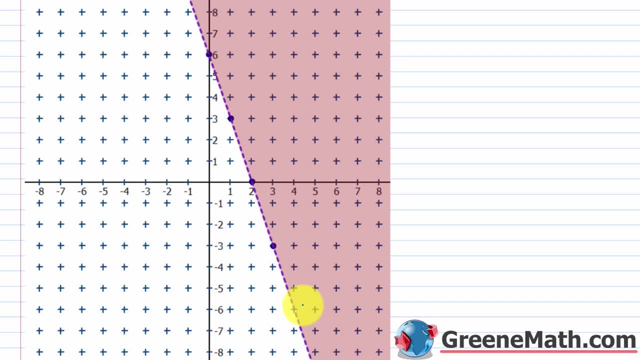 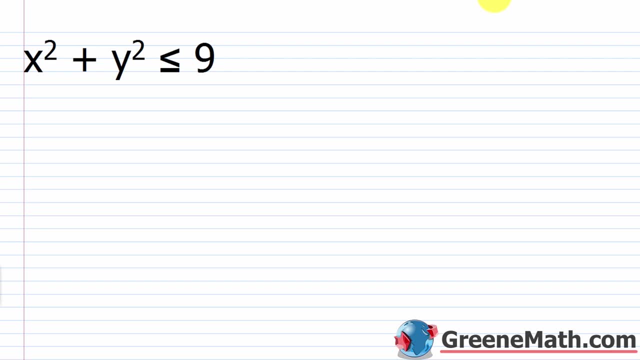 But anything above the line works as a solution to the inequality, And so it's part of our solution set. Alright, now let's jump in and look at our first example, where we have a non-linear inequality. So we have x squared plus y squared is less than or equal to 9.. 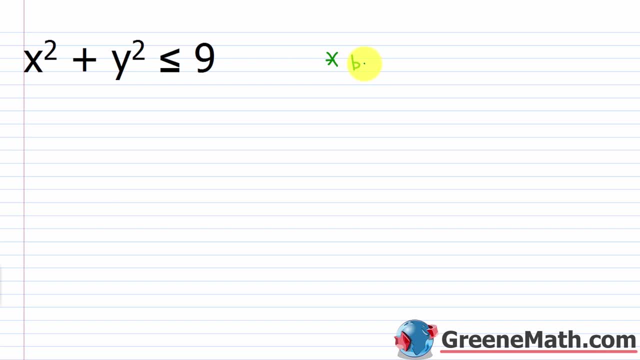 Again, the first thing I want to do is graph the boundary. So now, I'm not going to have a boundary line. In this case, if I replace the inequality symbol with equals, I'm going to have a circle, So the circle is going to be the boundary. 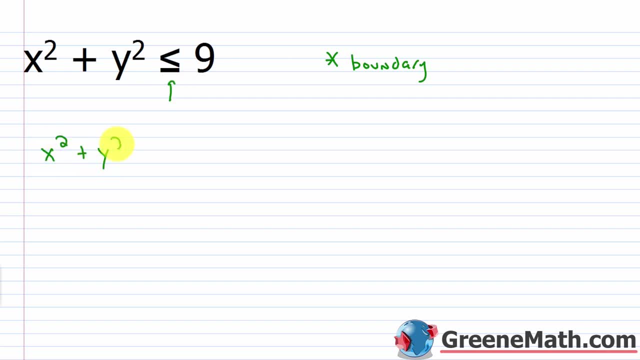 So let's do: x squared plus y squared equals 9.. Okay, squared equals nine. So this is a circle that has a center at the origin and that has a radius of three right. The square root of nine is three, So the center is obviously at zero, comma, zero. 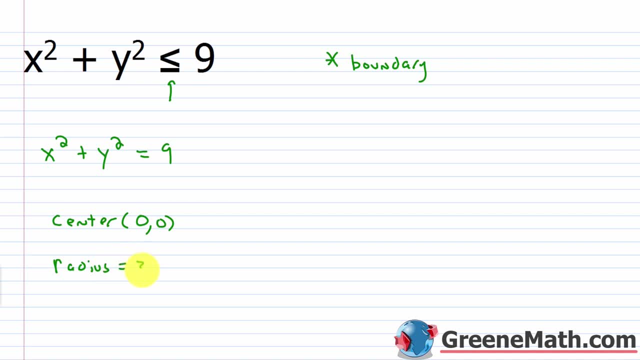 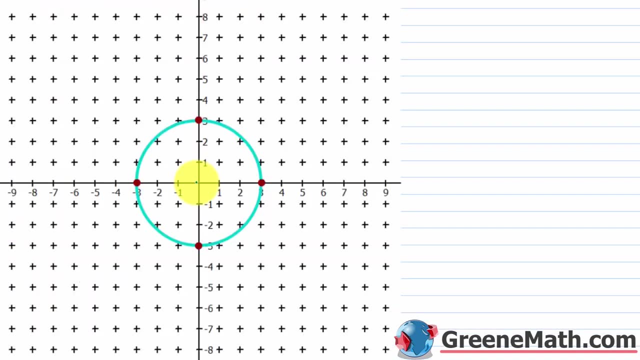 and the radius is three. This guy right here, remember this is a non-strict inequality. so I'm going to have a solid boundary. I go to my center and from the center I go three units to the right- make a point. three units down- make a point. three units to the left- make a point. 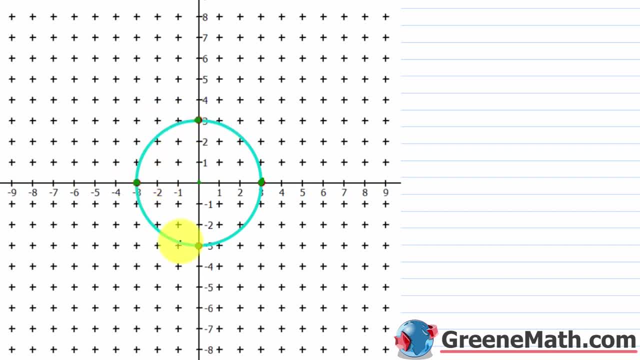 three units up, make a point. So I have my circle. I would obviously sketch the graph around those points And so, again, it's a solid graph because it's included in the solution. Now the next thing we want to do is use a test point. Let's use zero comma zero. It's not on the circle, It's the center. 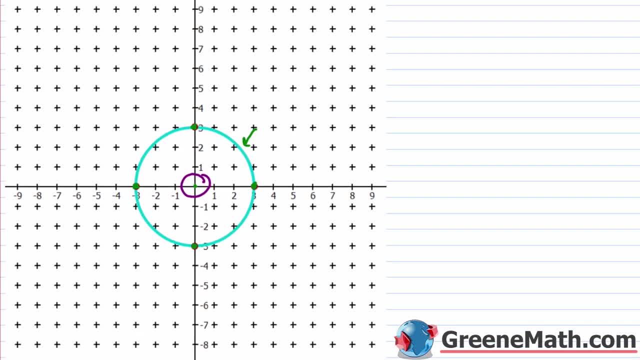 of the circle, but it's not on the circle. So zero comma zero, Let's go back up. So if I plugged in a zero comma zero, let's go back up. So if I plugged in a zero comma zero, let's go back up. So if I 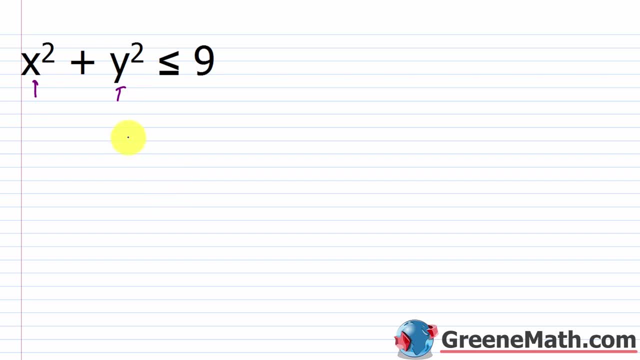 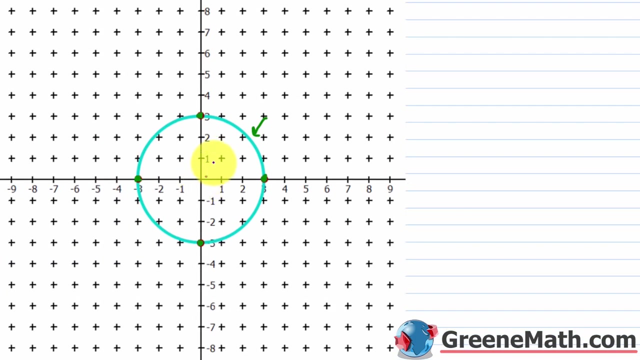 for x and a zero for y. what would I get? I would have: zero is less than or equal to nine, which is true, right, Zero is less than nine. So that tells me zero, comma zero lies in the solution region. So the solution region here is anything inside of the circle, Remember. 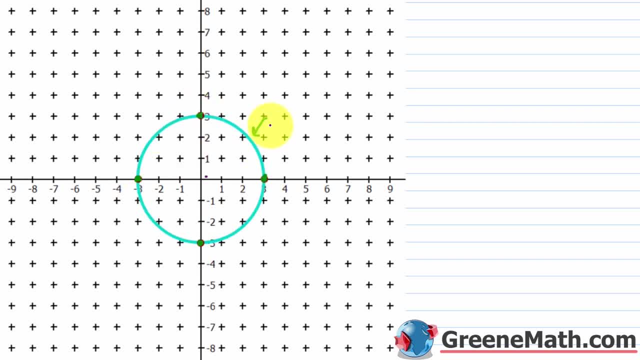 the circle is the boundary, So you're either on the inside of the circle or you're on the outside of the circle. In this case, since it's on the inside of the circle, I would shade everything inside of the circle. All of those points inside the circle would satisfy the inequality Again. 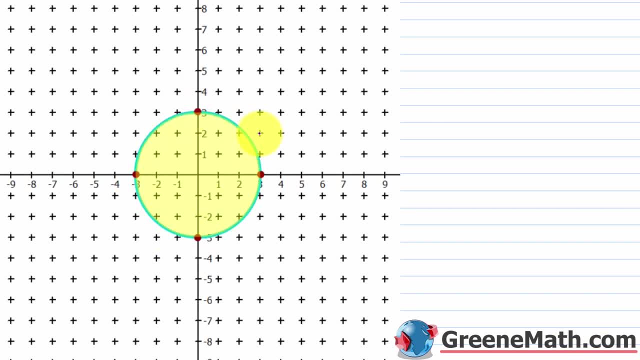 for a nice computer-drawn graph. you can see we have our circle Again. it's drawn as a solid circle because the circle itself is part of the solution set, And then the shaded area is everything inside of the circle. So this is the solution region, right, Everything inside that. 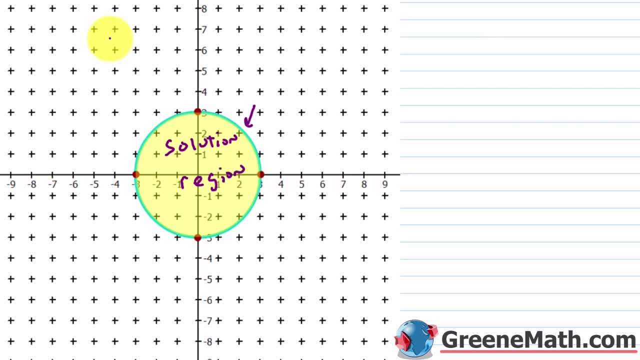 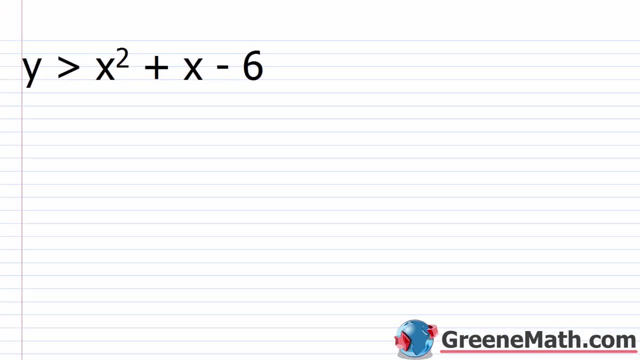 circle would work as a solution for the inequality, And then anything outside the circle would not work. right, That's the non-solution region. All right, let's take a look at another one. So we have: y is greater than x squared plus x minus six. So again, if I want the boundary, 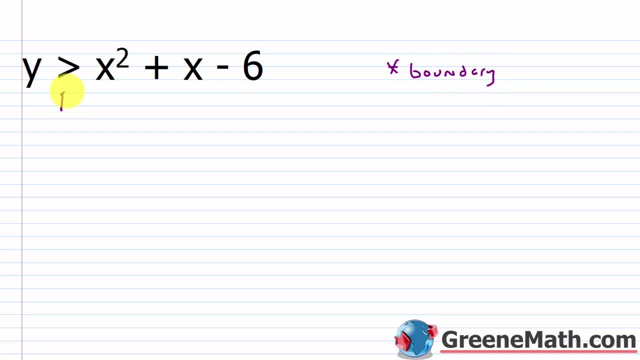 the boundary. what do we get? We replace this with equals. We'd have: y is equal to x squared plus x minus six. This is going to be a parabola. Now, it's been a while since we worked with parabolas- It was a few sections ago- But we should kind of remember that we don't have to. 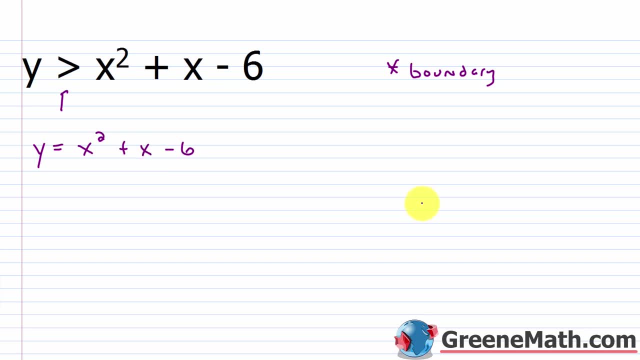 remember how to graph a parabola. It's one of those things that you really don't forget. The first thing you want to do is find the vertex And basically the formula for the vertex, in case you forgot. it occurs at the point negative b over 2a, comma f of negative b over 2a. 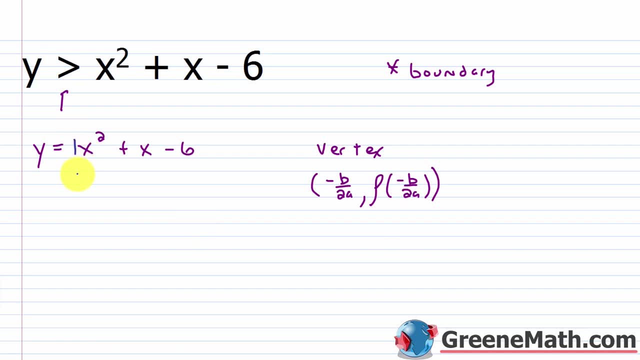 So what is a and what is b? Well, in case you forgot, a is going to be the coefficient right here for x squared, So this is a, And then b is going to be the coefficient for x to the first one, So that's b. So in each case they're one. So I'd have negative b, which is negative 1,. 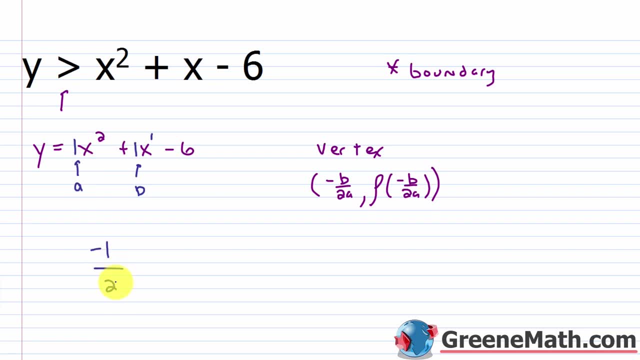 over 2 times 1, which is 2.. So basically negative b over 2a is negative 1 half, So negative 1 half. Now I want f of negative b over 2a. I know negative b over 2a is negative. 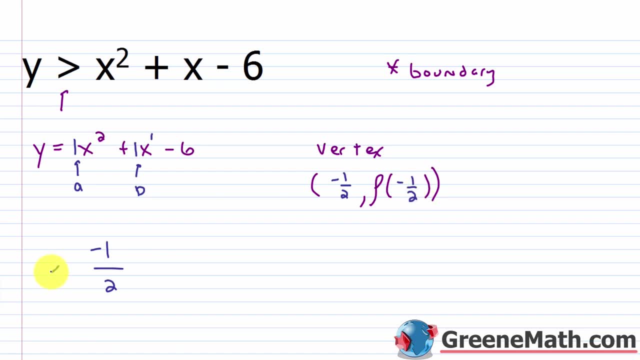 1 half. So I want f of negative 1 half. What is that? It's basically where I just plug in a negative 1 half for x and I evaluate. So this would be negative 1 half squared plus negative 1 half minus 6.. So let's see what we. 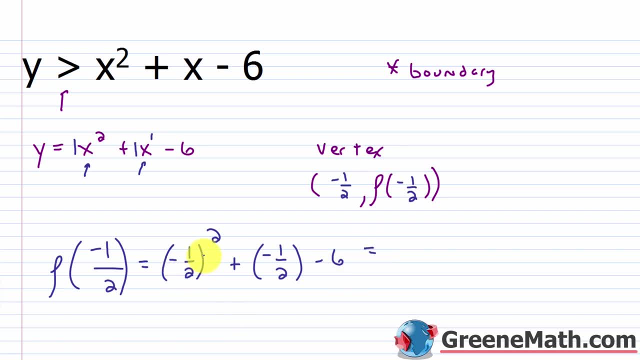 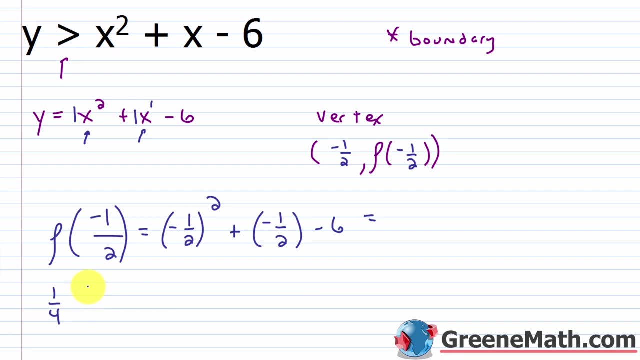 get with this. So negative 1 half squared would be 1 over 4, or 1 fourth. Then you'd have plus or you could say minus 1 half. I want to get a common denominator going now, So let's multiply. 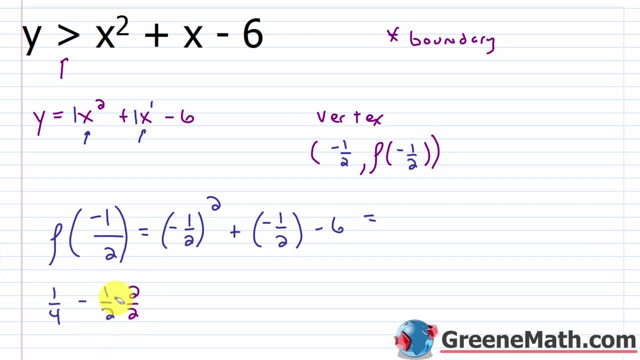 this by 2 over 2.. We could say this is minus 2 fourths. Then, lastly, we have minus 6.. But again, let's get a common denominator going. We'll multiply 6 by 4 over 4, and we'll have 24 fourths. So 1 minus 2 is negative 1. And then negative 1 minus 24. 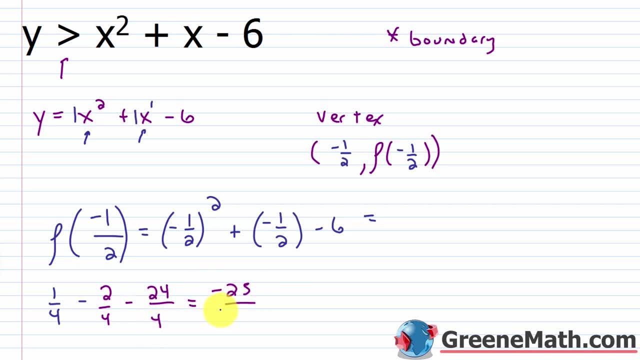 is negative 25.. This is over the common denominator of 4. So let's replace this with negative 25. fourths, We can erase all this. So now, generally when we graph a parameter, we want to get 3 points going. So we have our vertex, In this case, because the parabola opens. 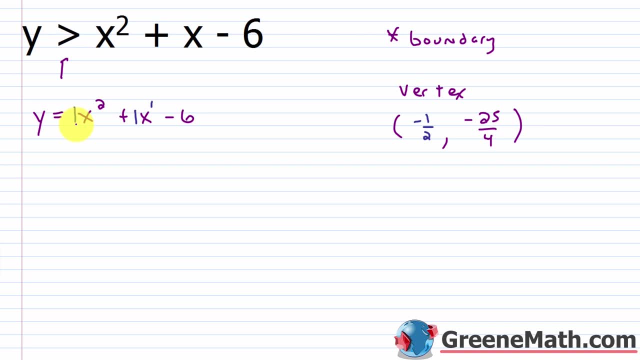 up. we know the vertex is going to be the lowest point, So it would look something like this. So we want to try to find the x-intercepts If we have those- in some cases we don't. we want to try to. 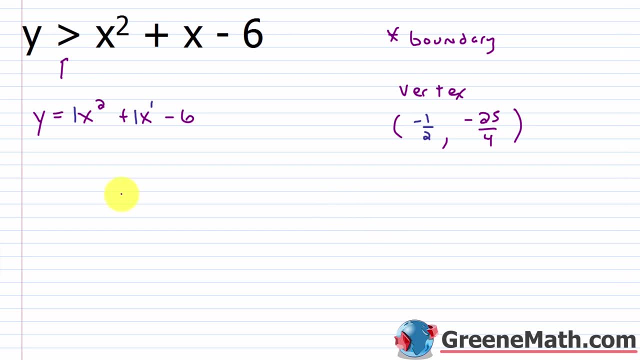 find the y-intercept. So let's take a look For the y-intercept. I can just replace x with 0. What would I have? 0 squared is 0. Plus 0 is 0. So you basically have 0 minus 6, which is negative 6. So if x is 0, y is negative. 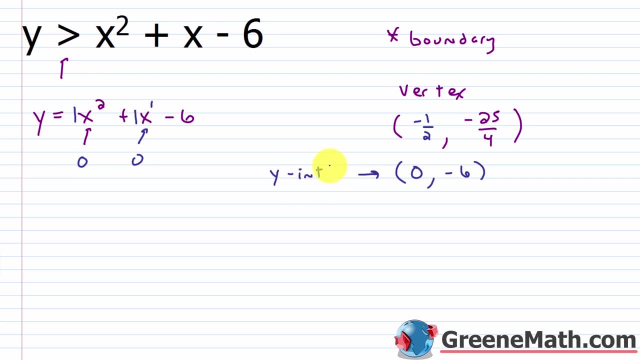 6. This is your y-intercept. What about the x-intercepts? So the x-intercepts? Well, in this case you're going to have 2 of them If I replace y with 0, and I solve the resulting equation. 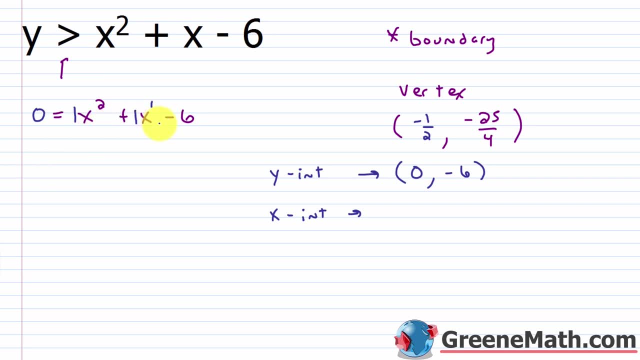 I get my x-intercepts So you can factor this right side here. I'm going to kind of flip it around and say this is 0. And I'm going to put in the x-intercepts. So I'm going to put in the 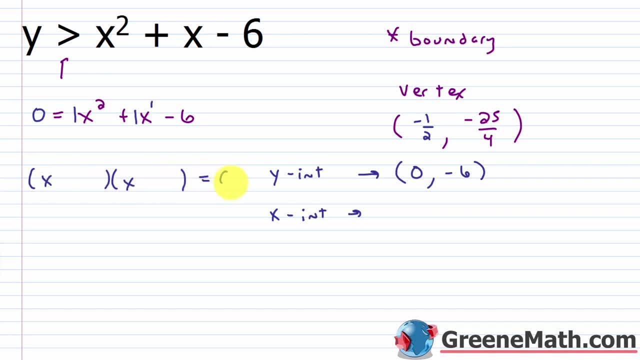 is x here and x here, and I'll set it equal to 0 over here. and give me two integers whose sum is 1 and whose product is negative 6. Well, you could do positive 3 and negative 2.. So, if I have the 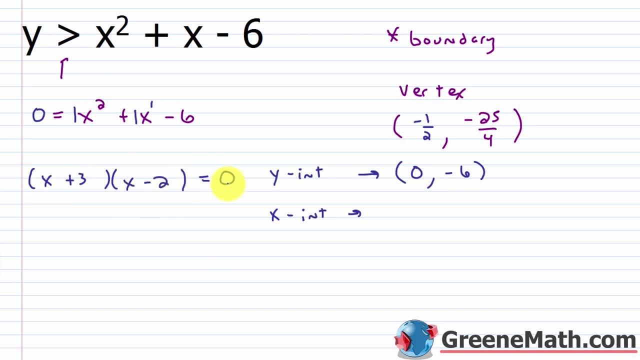 quantity x plus 3 times the quantity x minus 2, and this is equal to 0. I can set each factor equal to 0. So x plus 3 equals 0. the solution to that would be: x equals negative 3.. So one x intercept would: 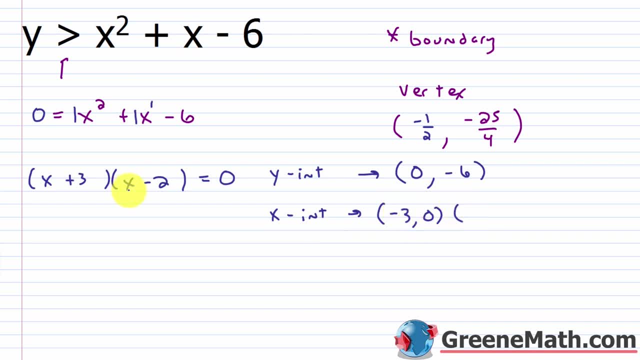 be negative, 3 comma 0.. The other one: if I set x minus 2 equal to 0, the solution would be x equals 2.. So the other x intercept would be 2 comma 0.. All right, so now that we have those, let's go to. 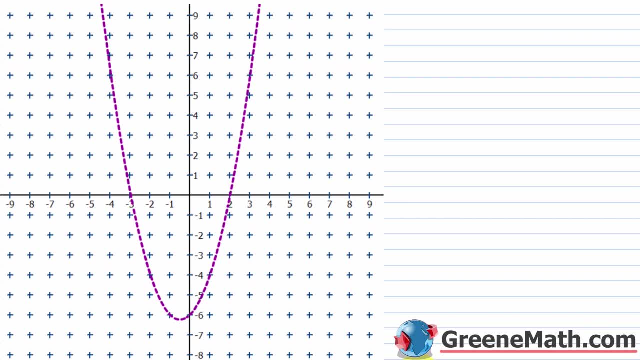 our coordinate plane. All right, so the first thing I would do is identify the vertex which is going to be right here. Basically what it is: it's negative one half. negative one half, which is about right here. comma: negative 25 fourths, which is about right here. All right, you think about. 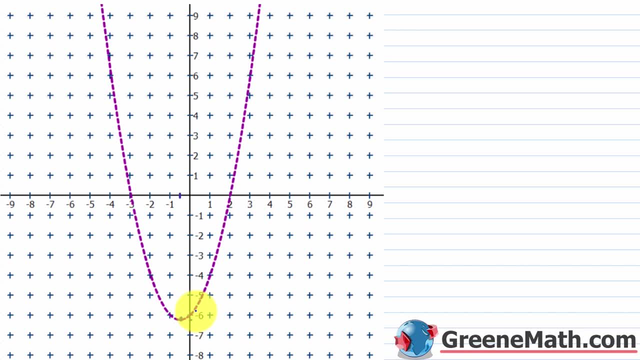 negative 1 half, which is about right here. All right, so now that we have those, let's go to our coordinate plane. All right, so now that we have those, let's go to our coordinate plane. All right. 24 fourths is negative 6. So you add another fourth to that in the negative direction. 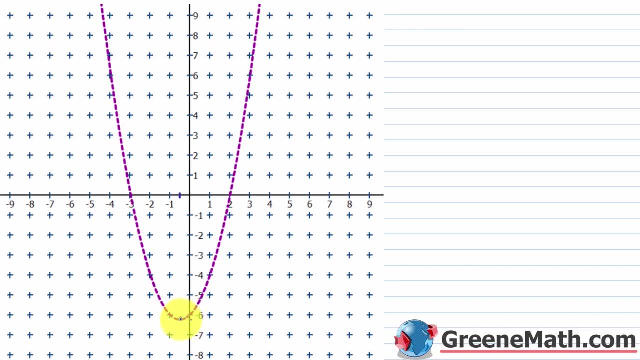 So you're going down by another fourth. So again, that's about right there. So this is about our vertex, right there. Then our y intercept occurred right here at 0 comma negative 6, and our x intercepts occurred at 2 comma 0 and negative 3 comma 0.. Now we graph the parabola and again: 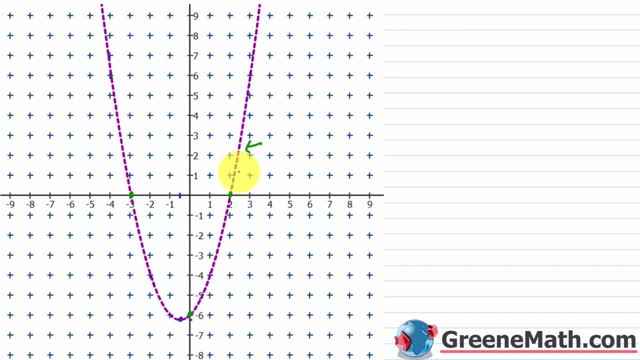 notice that this guy is graphed as a dashed parabola. That's because our inequality is a strict inequality, All right. so if I have a dashed parabola and I have a dashed parabola, I have a not part of the solution. Now we want to grab a test point, something that's not on the parabola. 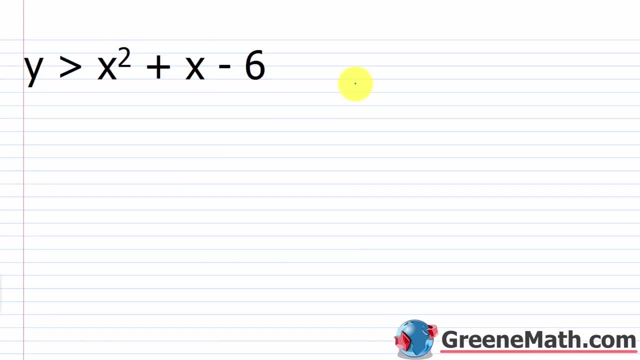 0 comma 0 is available, So let's check it. So our test point is 0 comma 0.. So I plug in a 0 for each x and a 0 for y. Now we get that 0 is greater than this is all gone negative 6.. 0 is greater. 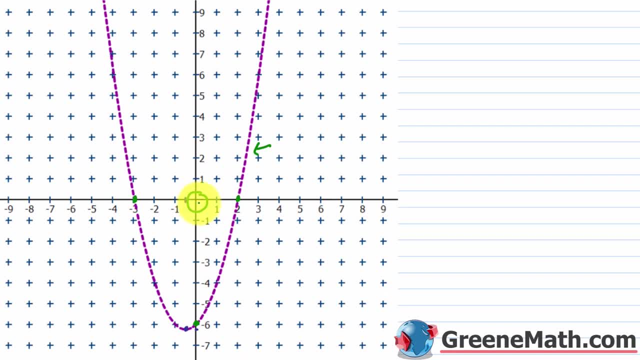 than negative 6. This is true. So that tells me that 0 comma 0 lies in the solution region. So when we think about the two regions, we're going to have to think about the two regions. So we're going to have to think about the two regions here. One would be inside the parabola and one 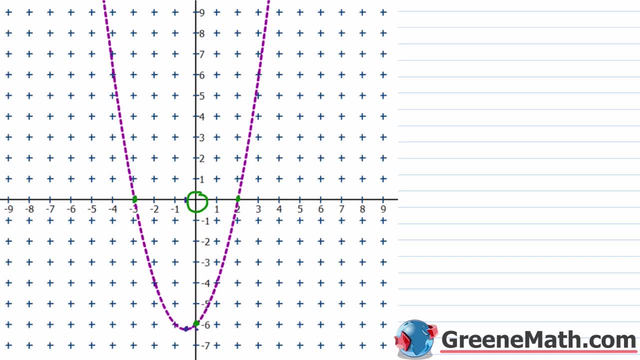 would be outside the parabola. Remember, the parabola is the boundary: It's separating the solution region from the non-solution region. So everything inside the parabola would work as a solution for my inequality. And then here's a computer generated image. Once again, you have a. 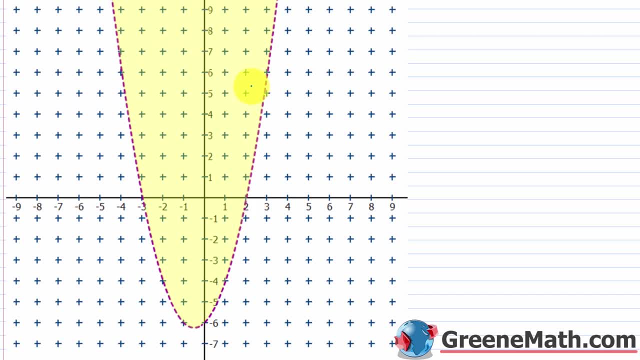 dashed parabola to show it's not part of the solution. And then everything inside of the parabola is shaded to indicate that this is the solution region. Anything outside the parabola will be in the non-solution region. So let's take a look at one. 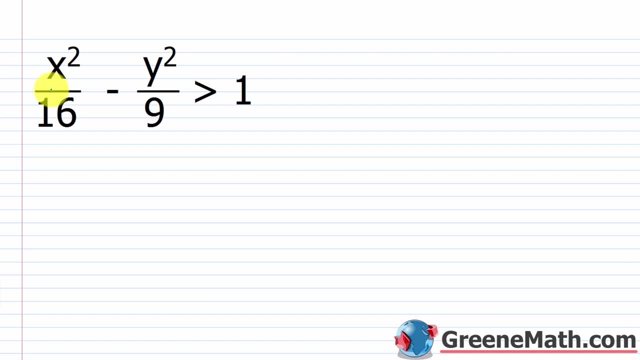 more of these and then we'll look at some systems. So we have x squared over 16 minus y squared over 9 is greater than 1.. So again, the first thing we're looking for is the boundary. So if I had x squared over 16 minus y squared over 9 is equal to 1, I'd be looking at a hyperbola again, because 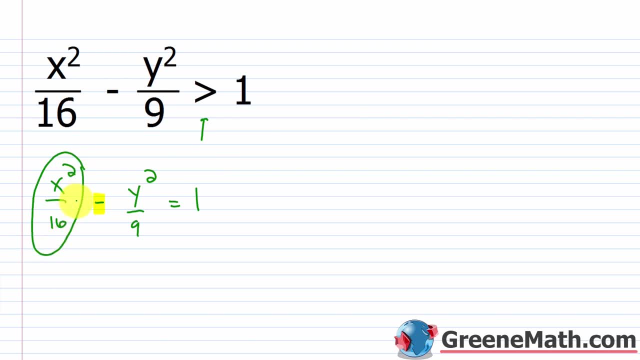 of the minus sign there And then again, because this is the positive one, I'd be looking at a non-solution region. We know this is a horizontal hyperbola and specifically, it's a horizontal hyperbola that is centered at the origin. So I know in this case I won't have any y intercepts. 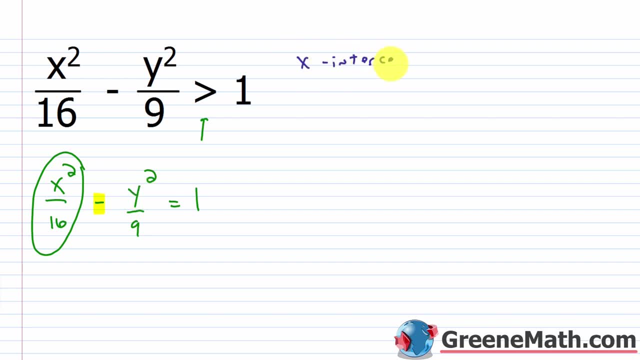 I'll just have x intercepts. So to find those it's very, very easy. We know y is 0 in each case and the shortcut is just to take this denominator here and take the principal and the negative square root of that Plus or minus. the square root of 16 is plus or minus 4.. So the x intercepts. would occur at 4.. And then we have x squared over 16 minus y, squared over 9 is equal to 1.. So we know y is equal to 4.. So now we have x squared over 16 minus y, squared over 9 is equal to 1.. So 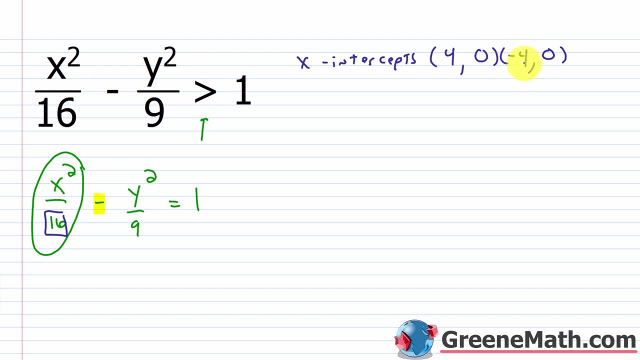 we know y is equal to 4.. So now the next thing you want to do: you can either find your asymptotes and then graph it that way, or you can find the rectangle and then from the rectangle you can extend from the diagonals to find your asymptotes. So however you want to do it, I'm just going to do. 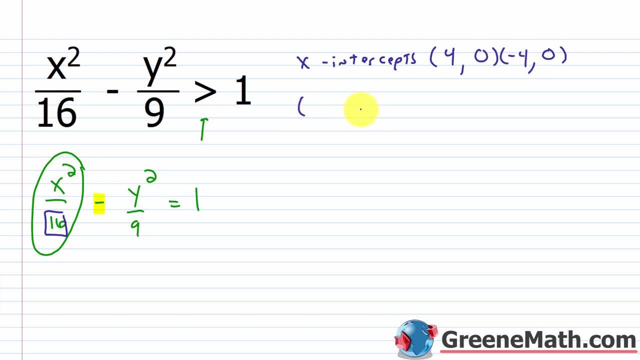 everything. so you have a complete understanding. The rectangle: there's four endpoints and I want you to remember how we go about getting those. So everything is looking at the denominators right and making sure that we're getting everything. So we're going to look at the. 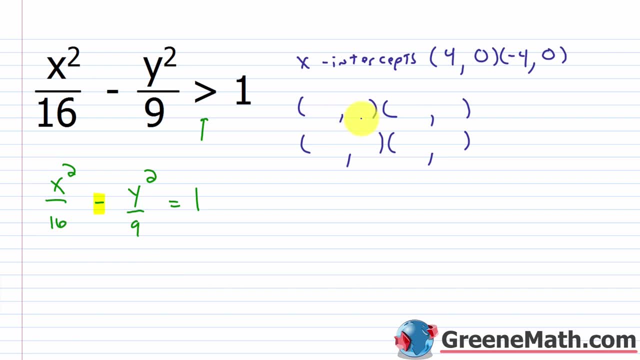 messing with the square roots. So it's x comma y. So I look underneath x squared, I have 16, pick the square root of that, I get 4.. I look underneath y squared, I have 9, pick the square. 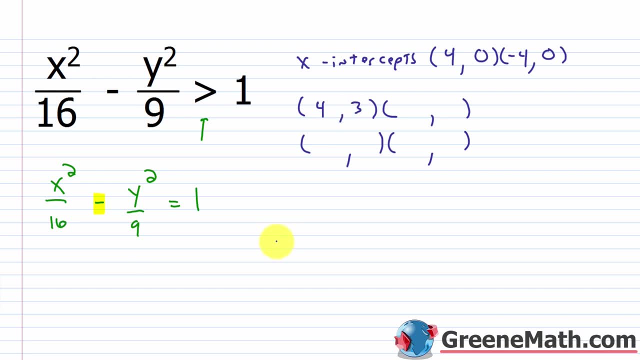 root of that, I get 3.. That's my x comma y, to kind of get things started. Then I do variations of that. So I'm going to do negative 4 comma 3,, I'm going to do 4 comma negative, 3, and then negative. 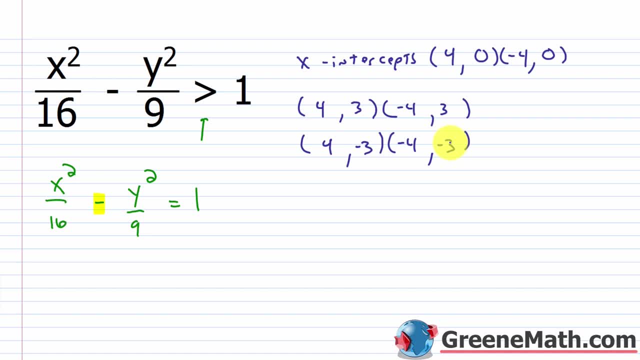 4 comma, negative 3.. So that's my fundamental rectangle. Again I can extend from the diagonals and get my asymptotes If I want the equations for the asymptotes. it's: y equals plus or minus. your slope is rise over run For the rise. take the square root of what's underneath y squared. 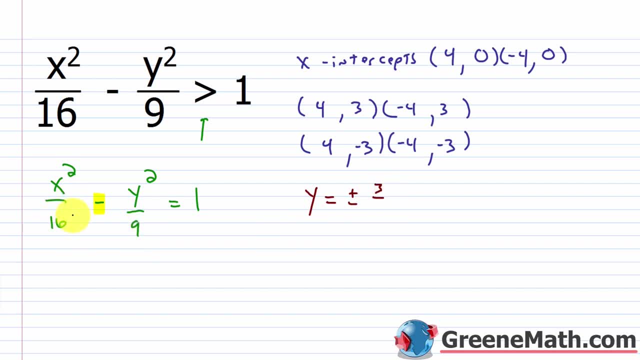 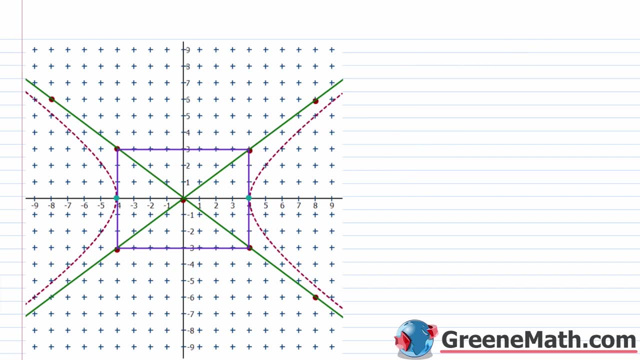 the square root of 9 is 3.. For the run, take the square root of what's underneath x squared, the square root of 16 is 4.. So y equals plus or minus 3 fourths x. So we have everything. 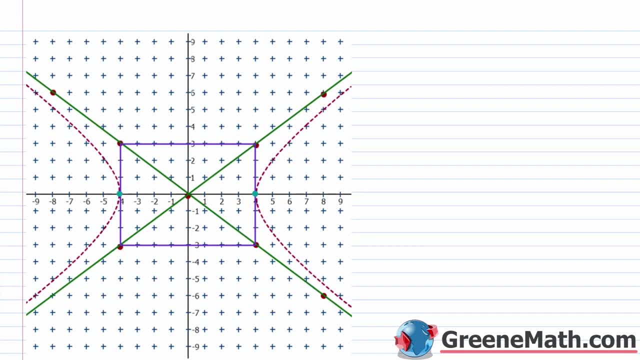 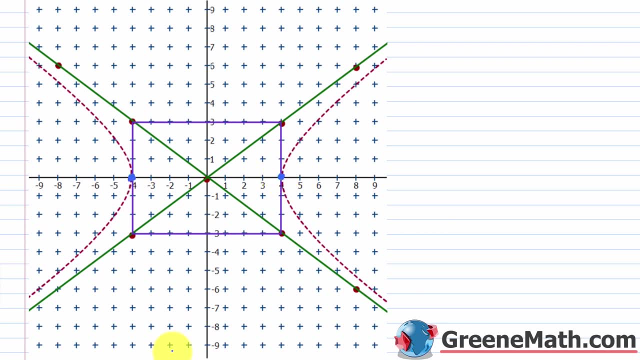 pre-drawn. but again, you can kind of follow along. We know that the intercepts occurred at 4 comma 0. We know that the points for the fundamental rectangle were 4 comma 3, negative 4 comma 3, 4 comma negative 3, and negative 4 comma negative 3.. Again, if we wanted to, we could. 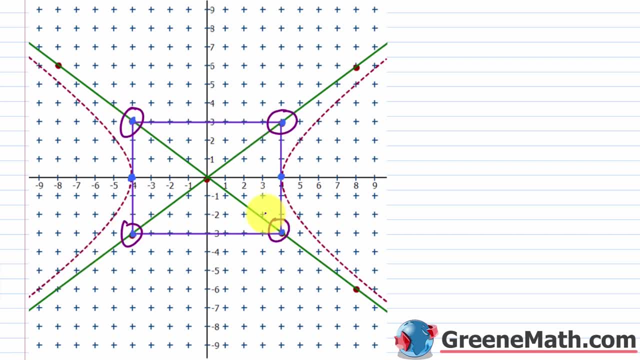 extend the diagonals here and get our asymptotes. Those would be your two lines Or you could graph it with the equations. we found: y equals plus or minus 3 fourths x. So if I start at the origin, if I went up 3,. 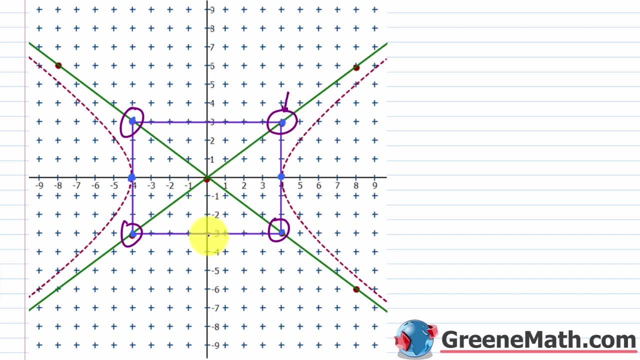 into the right 4, I'd have that point. Or if I went down 3, into the left 4, I'd have that point. So that's one line. If I start at the origin and I went up 3, into the left 4, that'd be that point. 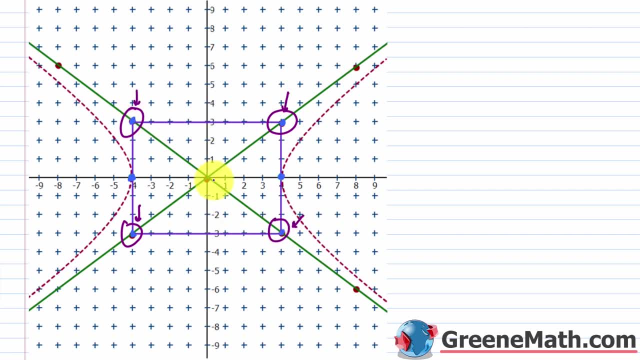 Or down 3, into the right 4,. that'd be that point. So, however you want to do it, you end up graphing the asymptotes, And so you have everything you need. Each branch of the hyperbola is going to. 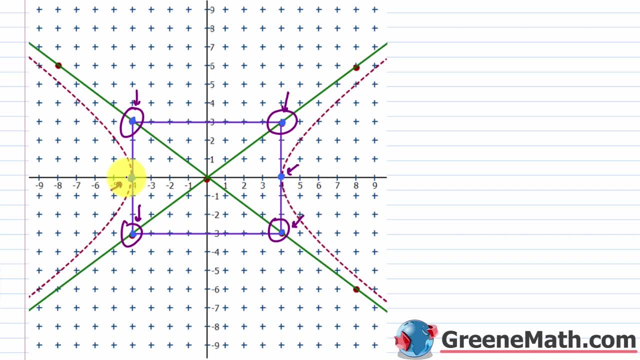 go through the intercept and it's going to approach the asymptote but not touch it. Now these guys, again you see that they're dashed and that's because we have a strict inequality. Now 0, 0 is available. It's not on either branch of the hyperbola. So if I use 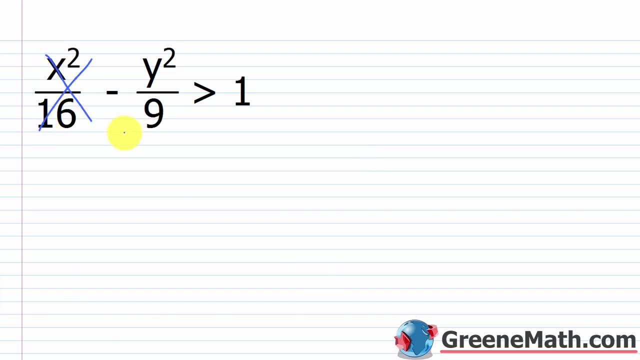 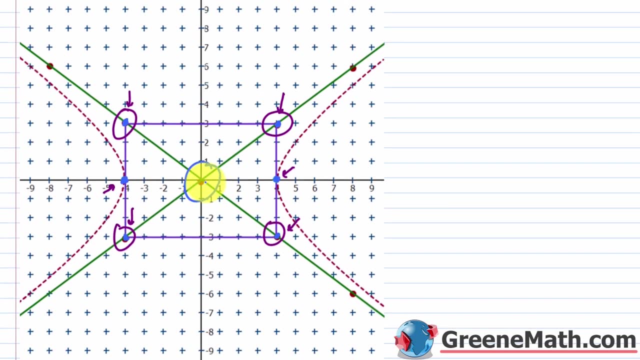 0, 0 as a test point. plug in a 0, that would be gone. this would be gone. You basically would have 0 is greater than 1, which is false. So that tells me that 0, 0 is in the non-solution region. 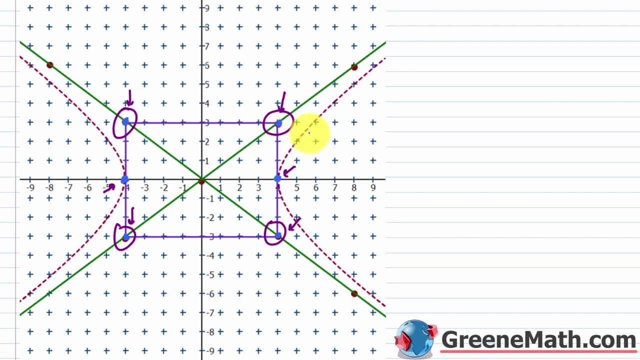 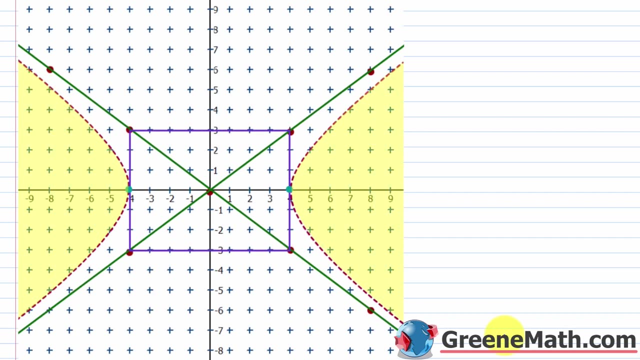 So what we would shade here is everything to the right of this branch right here and everything to the left. So if I go to the left of this branch here, that would give you the solution region for this inequality. Again, just to show you a computer-generated graph. you see, this is the 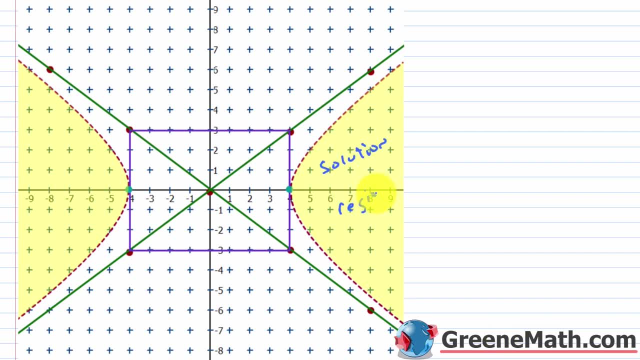 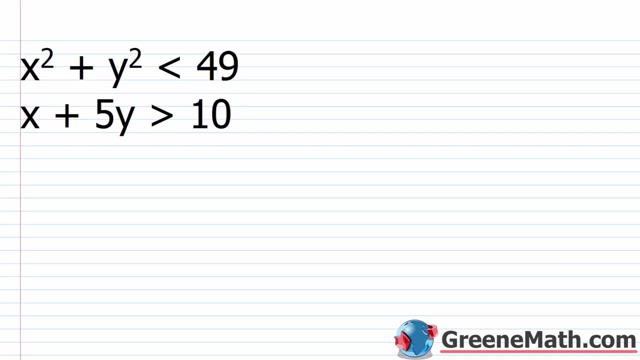 solution region along with this side over here. Anything outside of those areas that are shaded will not work as a solution in the inequality. All right, now let's look at a system of nonlinear inequalities. The concept of nonlinear inequalities is that nonlinear inequalities are 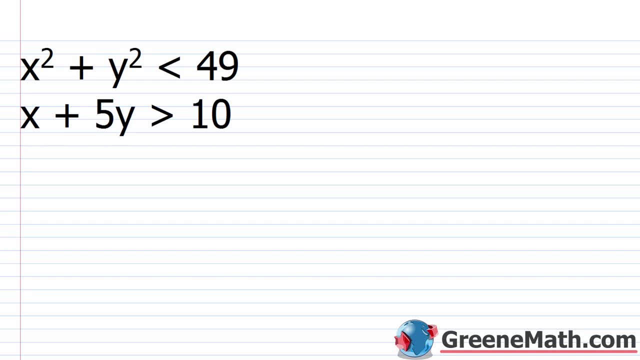 the same. All we're doing is graphing stuff. that's a little bit more tedious, So that's why it takes more time than when we work with just linear inequalities or systems of linear inequalities. So we have x squared plus y squared is less than 49.. Let's start out with this one. We know that. 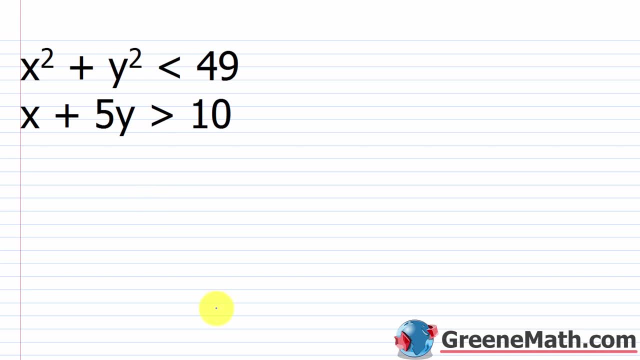 the boundary here would be a circle and we know the boundary would be dashed because this guy is strict. So it's x squared plus y squared is equal to square root of 49 is 7, so I might as well say this is 7 squared. So this is a circle, and I'm going to say that this is a circle and I'm going to 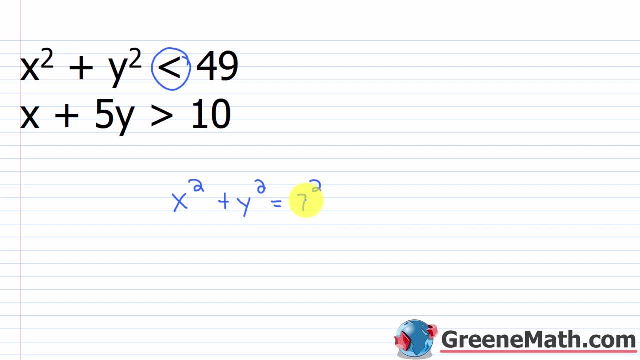 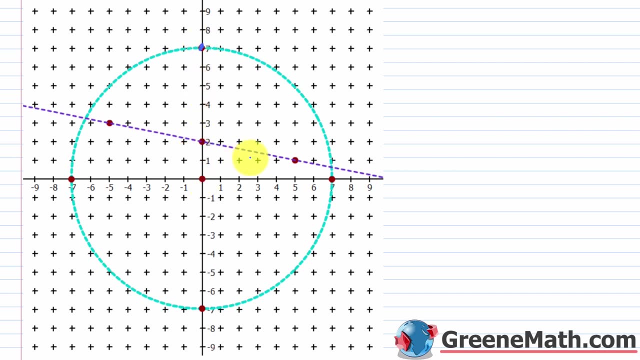 say that this is a circle that is centered at the origin with a radius of 7.. So let's go down here. So, centered at the origin, a radius of 7 means I go up 7 to make a point, the right 7 to make a. 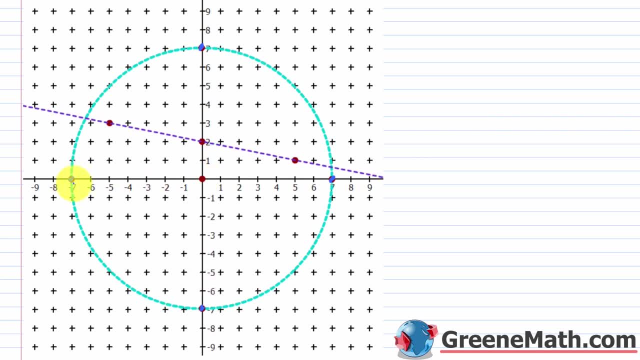 point down: 7 to make a point. the left 7 to make a point. Again, graph my circle as a dash circle, because no point in that circle is part of the solution set For the test point. let's choose 0,. 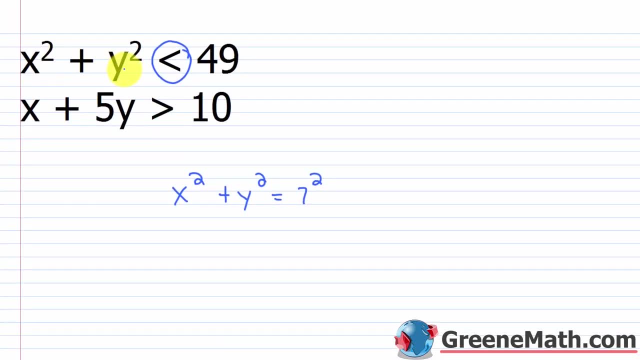 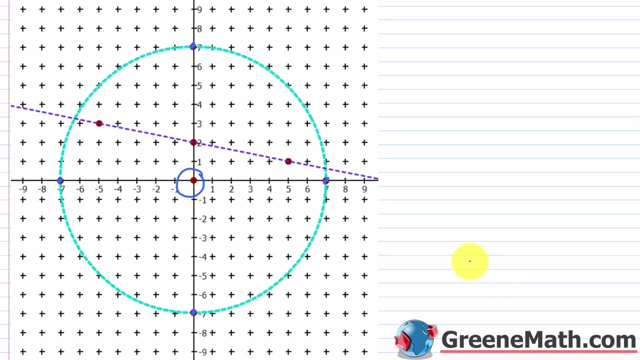 0. And if I had a 0 for x and a 0 for y, I would have 0 as less than 49, which is true. So that tells me that the solution for that first inequality would be that I would shade everything inside of the circle. But I'm not done, because it has. 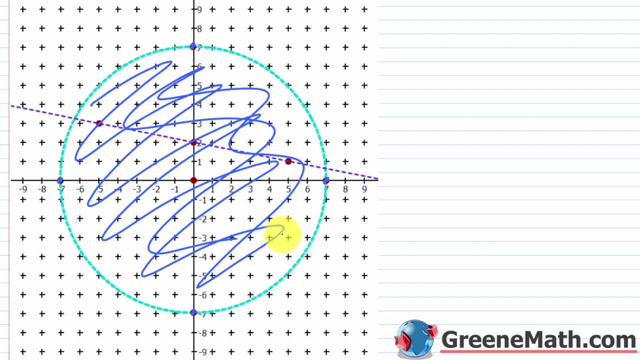 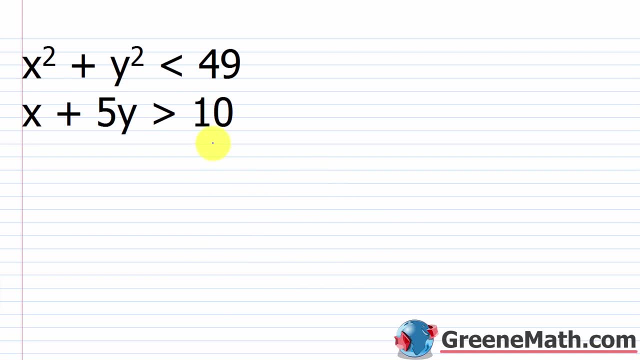 to satisfy both the first inequality and the second inequality. So let's go back up, Let's think about this second inequality here, And I'm just going to label this so I can refer to stuff: This is inequality one and this is inequality two. So let's work. 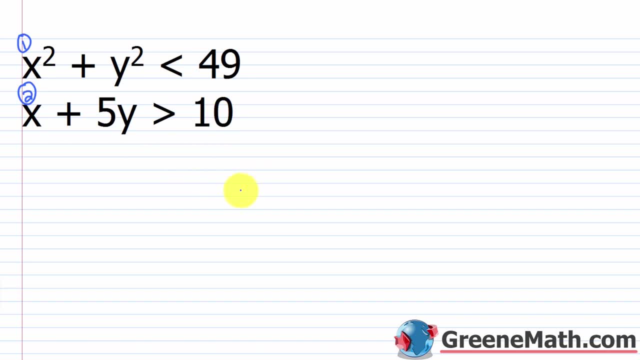 on inequality two now. So this guy will be a line. when we make the boundary, x plus 5y is equal to 10. And again it's going to be dashed because we have a strict inequality. So let's solve this for. 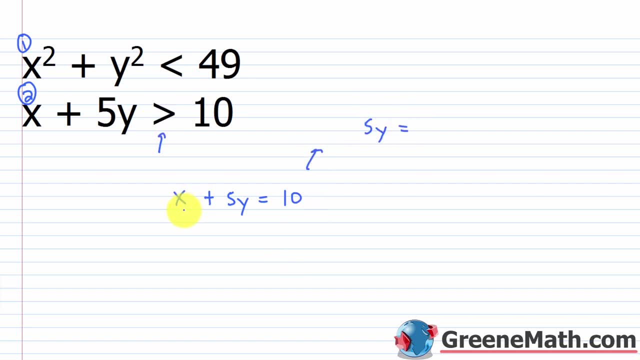 y, This would be 5y is equal to. I'm going to subtract x away from each side of the equation and then divide both sides of the equation by 5.. That would give me y is equal to negative 1. fifth, x plus 2.. 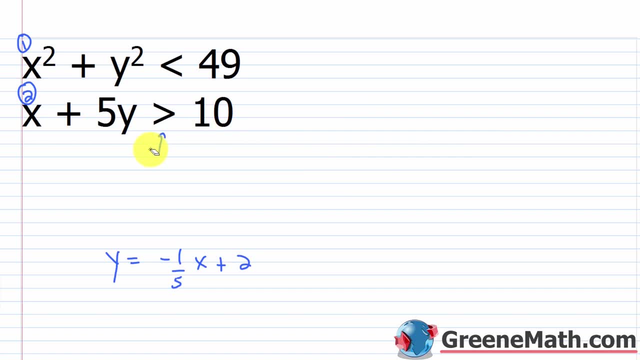 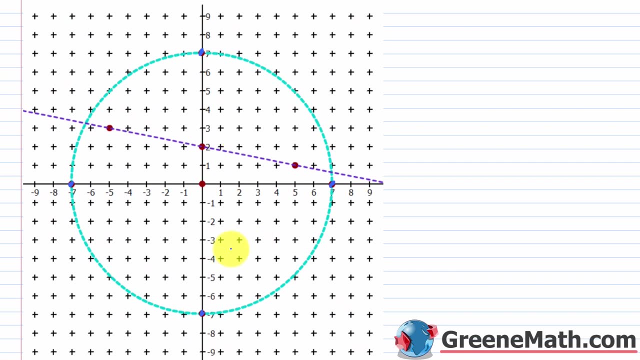 So my y intercept occurs at 0 comma 2, and my slope is negative 1 fifth. So my y intercept- let me just erase this real quick- My y intercept occurs at 0 comma 2,, right here My slope is: 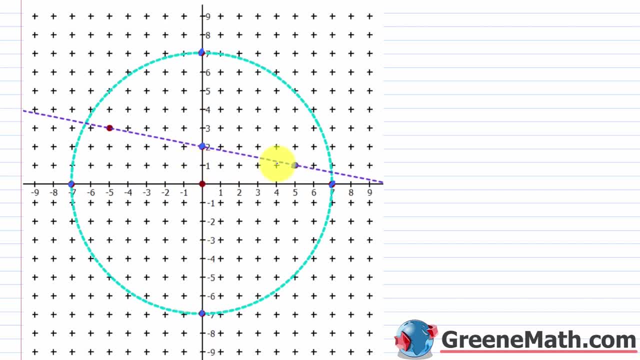 negative 1. fifth, So down 1 to the right 5, or I can go up 1 into the left 5.. So that's where that line came from. Again, it's dashed because it's not part of the solution. Now, where is our solution? 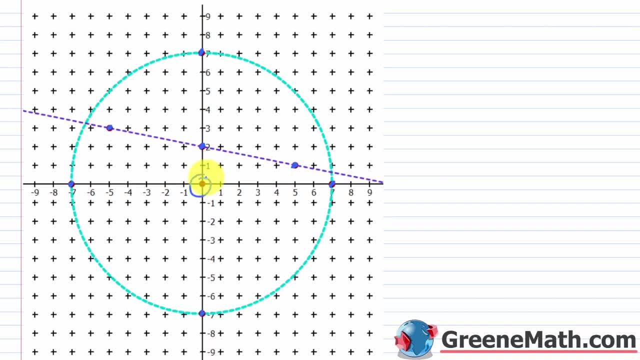 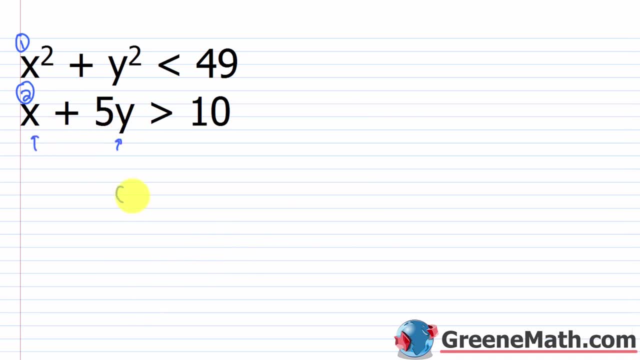 region for inequality number 2?. Take 0 comma 0, you can use that as a test point, And if I plugged in a 0 for x and a 0 for y, essentially I would have 0 is greater than 10, which is false, So 0. 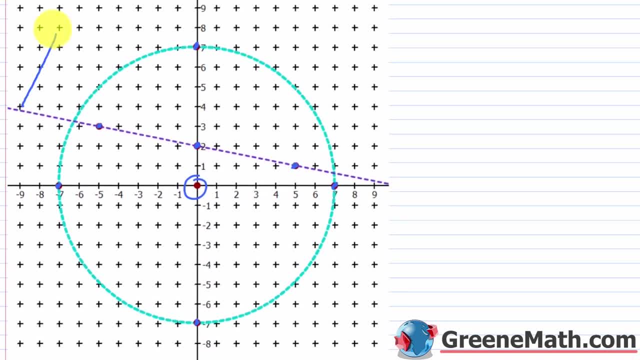 comma 0 is not in the solution region, So I would want to shade everything above the line. So let's think about this: We need the overlap of the two graphs. With inequality 1,, it was anything inside of the circle. With inequality 2,, it's anything above the line. So, essentially, the overlap of the two graphs. 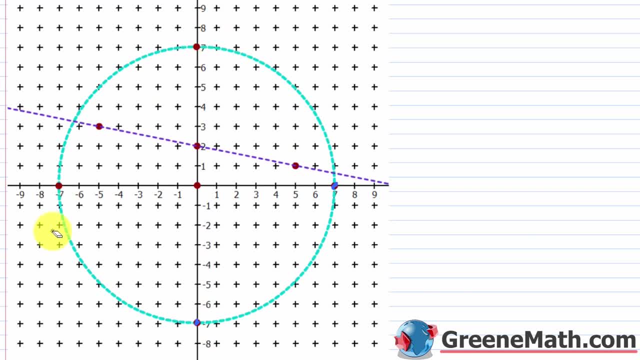 or the area of the coordinate plane that satisfies both would be anything above the line that is inside of the circle. So this section right here, And just to let you see what a computer does, you can see this graph is basically perfect. You have a dashed circle because it's not included. 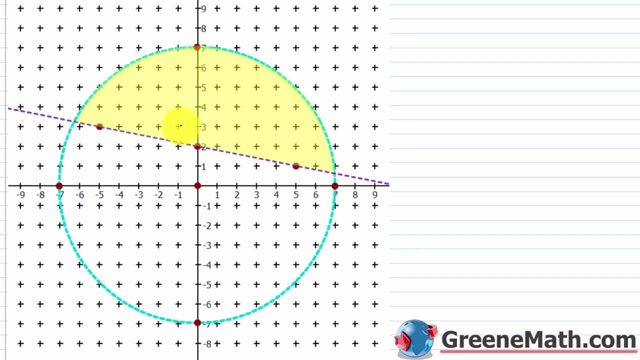 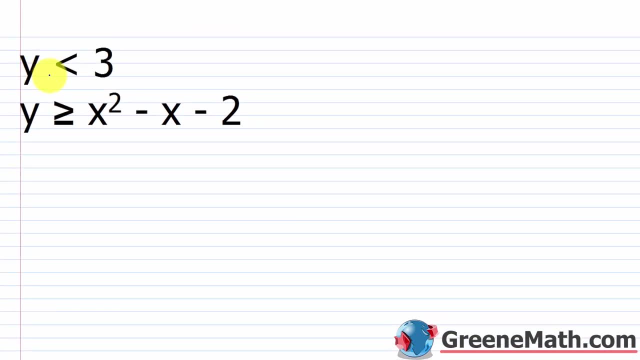 also a dashed line, Because it's not included. anything above the line that's inside of the circle is in the solution region. All right, let's take a look at one more. So we have y is less than 3.. We also have y is. 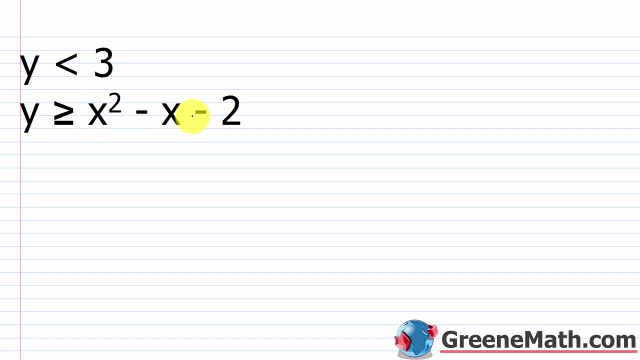 greater than or equal to x squared minus x minus 2.. So let's call this inequality 1 and this inequality 2.. For y is less than 3, it's a strict inequality, so the boundary line will be broken. But we're basically graphing as a boundary line: y equals 3.. 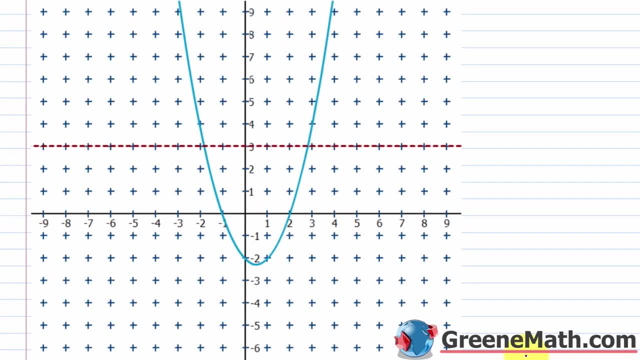 Now let's take a look: y equals 3 is a horizontal line, So really it's just this line here that crosses through 0,, 3 on the y-axis, But for every x value, y is equal to 3.. Now, in terms of where we 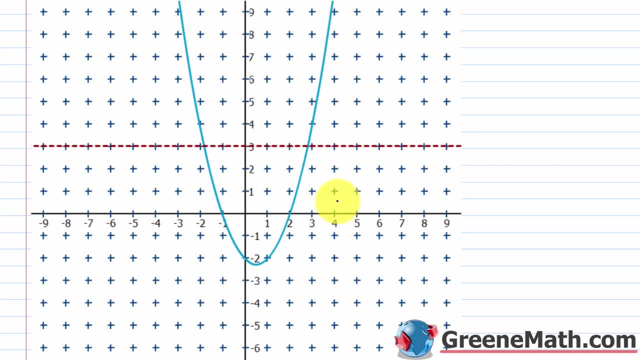 want to shade, y is less than 3.. So any value of y that's less than 3 works. So we would be shading below the line. So anything below the line works as a solution to that first inequality. Now let's take a look at the second inequality. This guy is a non-strict inequality, So the 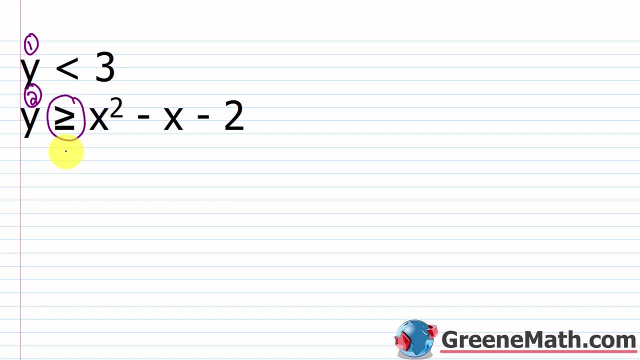 boundary will be solid right, And we're graphing a parabola here. You'd have: y is equal to x squared minus x minus 2.. This is a parabola that opens up, So we would want the vertex to start. 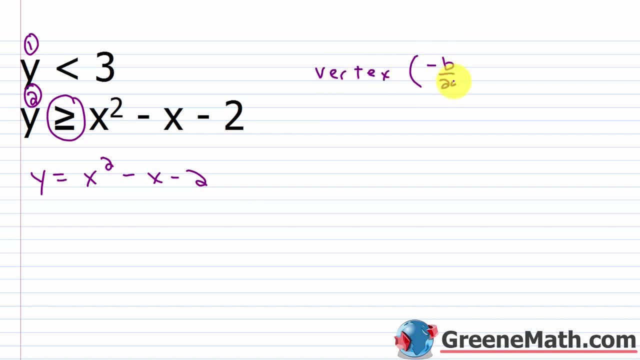 Again this occurs at negative b over 2a, comma f of negative b over 2a. So again negative b. b here is negative 1.. And a here is 1.. So the negative of negative 1 is 1 over 2a. 2 times 1 is 2.. So you'd have 1, half for negative. 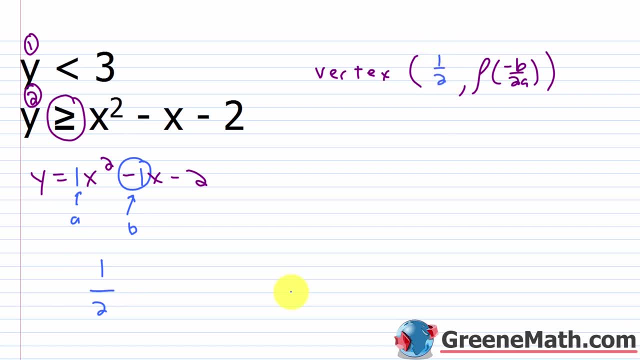 b over 2a. Then we want f of negative b over 2a. So we want f of 1 half. Let's erase all this. I'm going to plug in a 1 half there and also there. So f of 1 half is equal to…. you'd have 1 half squared, which would be one fourth. 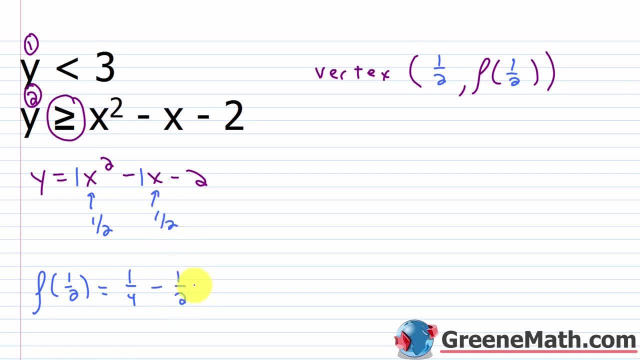 Then minus 1 times a half is a half. So let's get a common denominator and multiply this by 2 over 2. You'd have two-fourths there. Then minus 2 by 4 over 4. That would be minus 8 fourths. 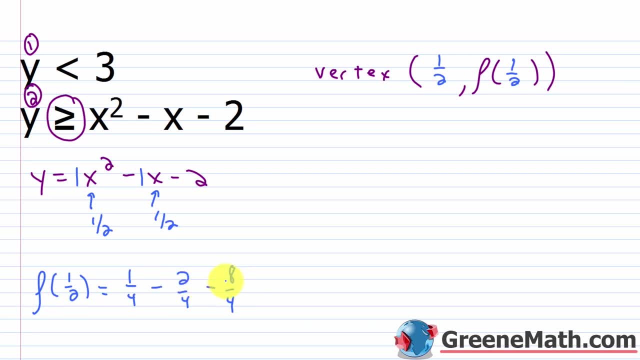 Gymn Jeong: 1, negative 1 minus 8 is negative 9.. So this would be negative 9 fourths. This, right here, is negative 9 fourths. Alright, so we have the vertex. What would our y-intercept be? 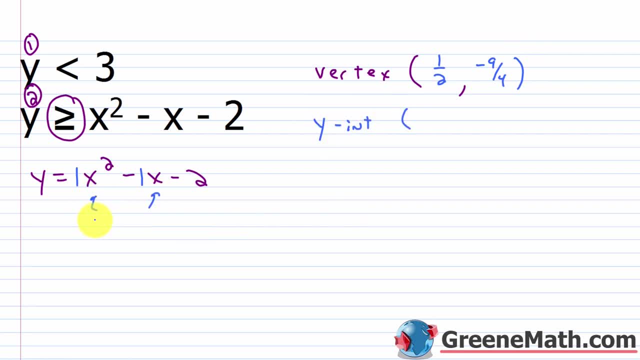 If I plugged in a 0 for x, I would get y equals negative 2.. What would our x-intercepts be? Well, we have 1,, 2, or 0.. I'd plug in a 0 for y, so I'd have x squared minus x minus 2 equals 0.. 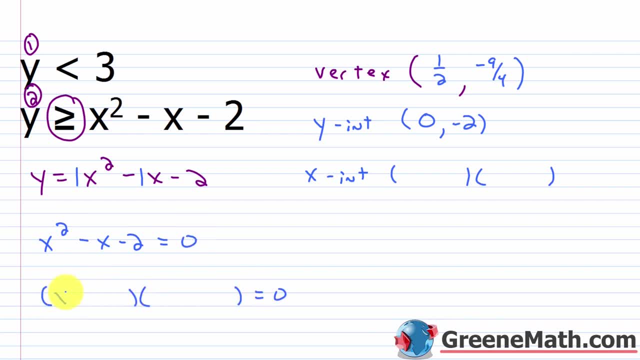 I can factor this and solve it, So we would have x here and x here. So give me two integers whose sum is negative, 1 and whose product is negative 2.. So you could do negative 2 and positive 1.. So if I solve each one of these factors, x minus 2 equals 0 has a solution of x equals. 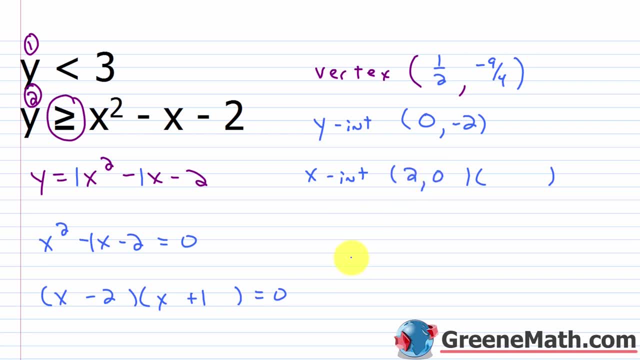 2. So 2, 0 would be one x-intercept. Then x plus 1 equals 0 has a solution of x equals negative 1. So negative 1, 0 is another x-intercept. So let's erase this and let's graph this. 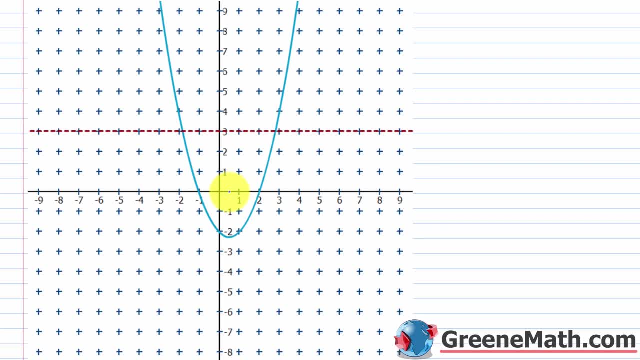 guy. I'm just going to erase what we've done already. So the vertex again is at a half comma negative 9 fourths. So right there. Then our x-intercepts. again we have 2, 0,.